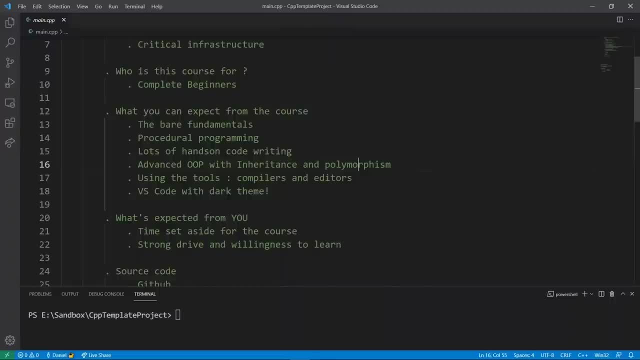 So if you don't know what a compiler is, if you don't know what an IDE is, we're going to make sure you understand these things And we're going to spend a lot of time using these things And by the time you're done with the course, you're going to be very comfortable using the tools. 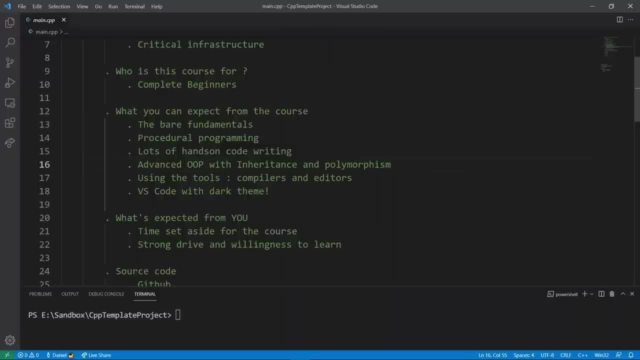 The editor of choice for the course is going to be Visual Studio Code, So that's an editor That is going to allow us to type in the code and give us some things like syntax highlighting. But we're going to be connecting our editor to a background compiler which is going to make sure our code is transformed to run on our computer. 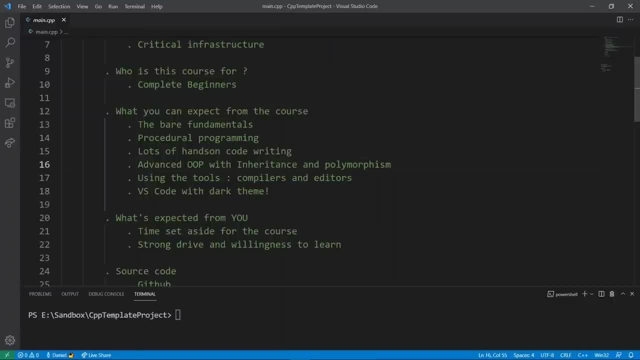 But don't worry about all that craziness right now. We're going to go in detail about these things. For now I just want you to have a bird's eye view on what you can expect from the course here Now. I hope you know what to expect from the course. 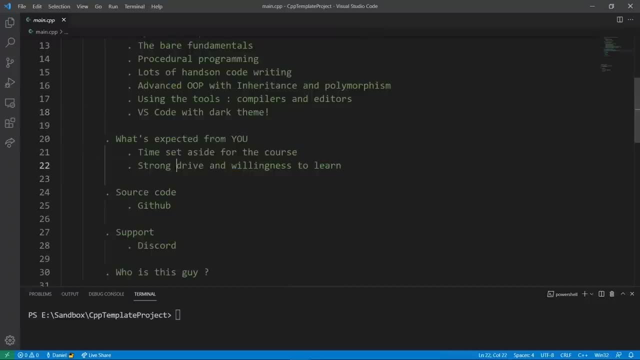 But I also expect you to be ready to take the course, And the requirements are really not that bad. The only requirement is that you have time set aside to really practice what you learn from the course here, And you need to have a strong drive and willingness to learn. 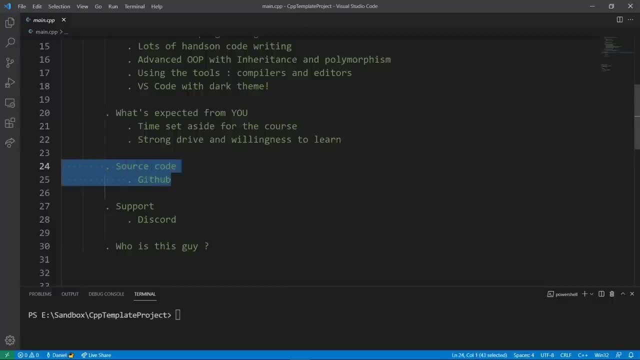 Now, if you want to follow along, I am going to share a link to the GitHub repository for the code I use in the course, So you can check that out and really follow along if you want. If you want some support, we have a Discord server. 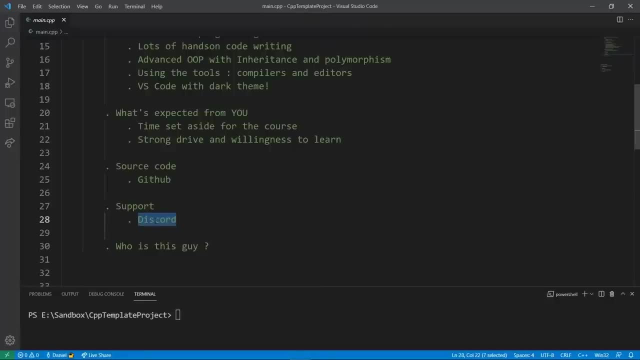 Dedicated for our students, So you can join and be part of the community. If you have a question, you can ask. But another thing I would encourage you to do is to also help others. So if you see somebody asking a question, try to help them. 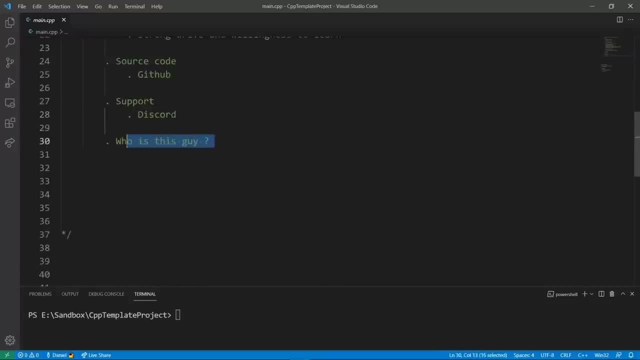 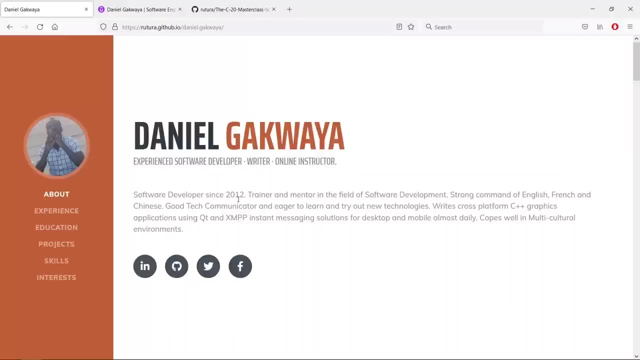 You're going to learn a lot that way. Okay, now that you know a bit about the course, let's talk about myself here. My name is Daniel Kakwaya. I am a software engineer. I have been writing code since 2011 or something. 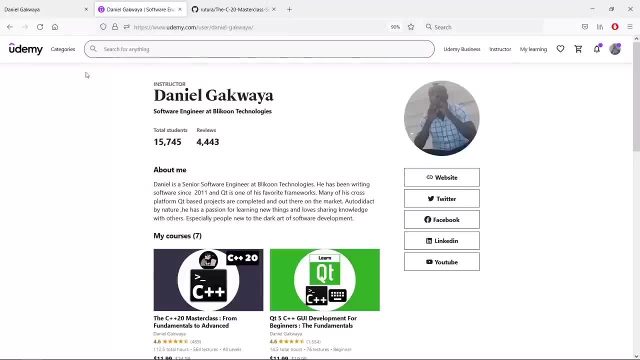 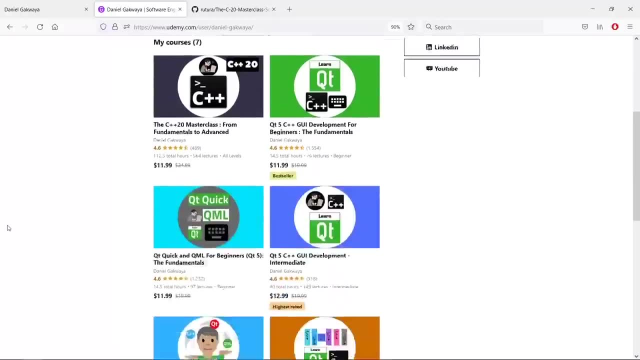 And I am a professional C++ developer. I do A lot of freelance work. I work for a few companies. I do all kinds of crazy things. I also like to teach others, So I have a few courses on Udemy. If you are interested in Qt, you can check these things out. 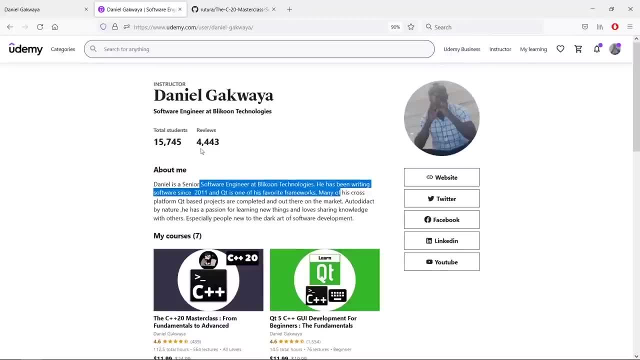 I also have a trending C++ course that you can check out, But don't feel the need to go and check this C++ course out, because a lot is covered in this YouTube course here. So that's really all about me. Okay, Now that you have an idea about the course we're going to head over in the next lecture. 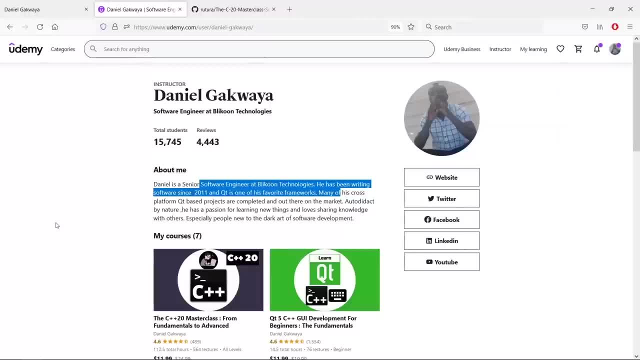 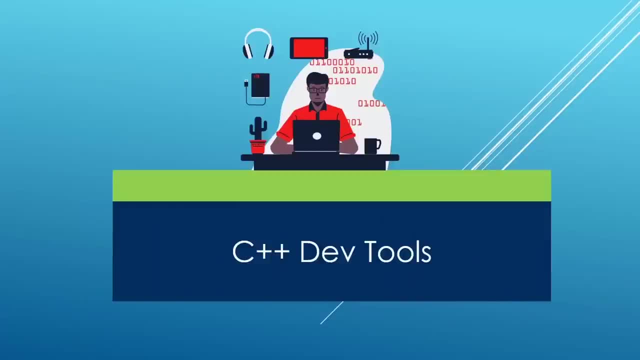 Okay, And learn about the tools we're going to be using throughout the course here. Go ahead and finish up here and meet me there. Welcome to this new chapter where we're going to be exploring the C++ development tools. you need to start writing your own C++ applications. 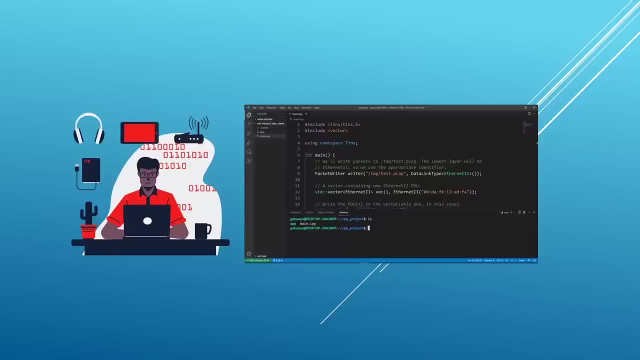 And you really need two kinds of tools. The first one is going to be an editor or an IDE through which you're going to be writing your C++ code. We are going to be using Visual Studio Code As an editor in this course, because it is very easy to install. 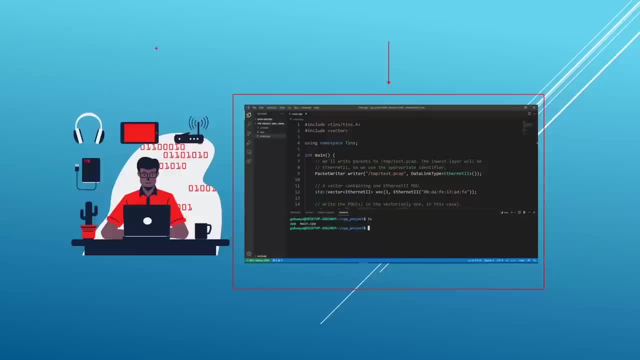 It is cross-platform, It is going to run well on Windows, Mac and Linux, and it supports a host of tools that are going to make your job easier as a C++ developer. But that's not to say you can't use your favorite IDE if you can, but Visual Studio Code is going to be our main editor in this course. 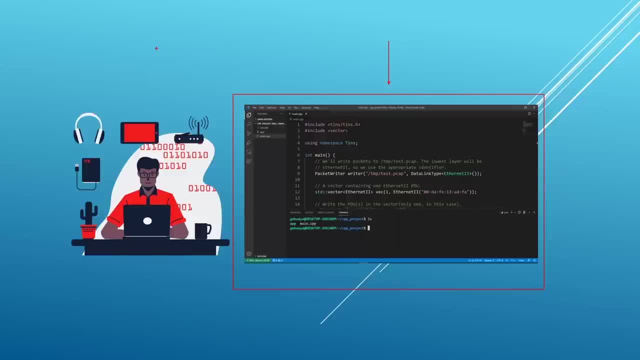 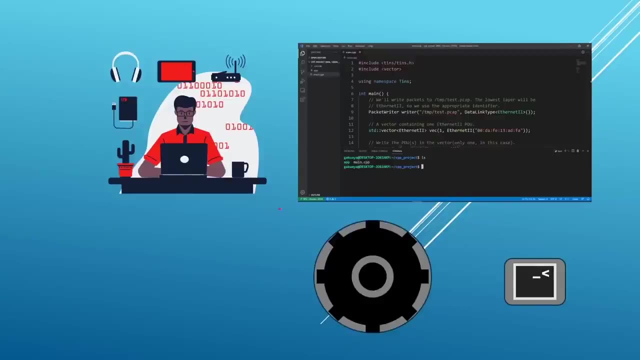 So I would recommend installing it to be able to follow along with what we do here. Now, after we have an IDE For an editor in place, we will need a compiler, and a compiler is a piece of software that takes the code we write in the editor and compiles that into code that can directly run on the hardware or binary executable format. 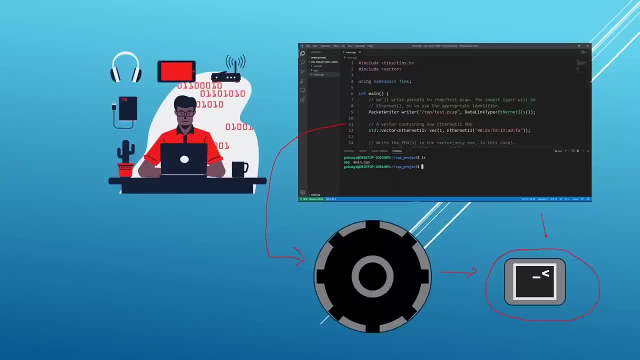 So this is what we're going to be doing here. We're going to be typing our code in an editor like Visual Studio Code. We're going to be kicking off a process to compile our program And this is going to turn our program. 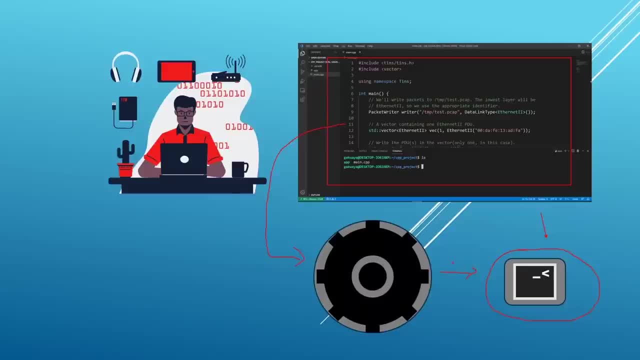 And to a format that can run it directly on the hardware. So, for example, if you are on a Windows machine, you're going to generate a binary executable that can directly run on Windows. If you are on Linux, we will generate a binary that can run on Linux. 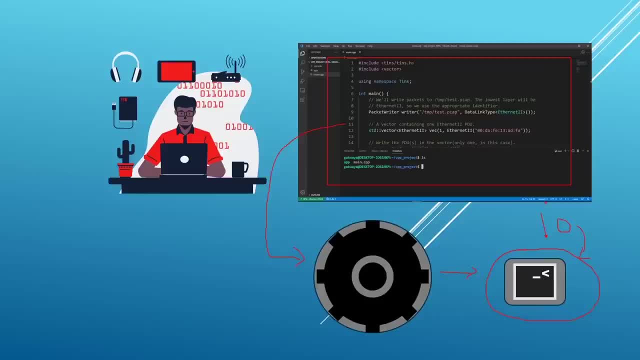 And the same concepts can really extend on Mac or any other kind of operating system you might be working on with the course here. So we need two tools. We need an IDE or an editor and a compiler, and the tools you install are going to be. 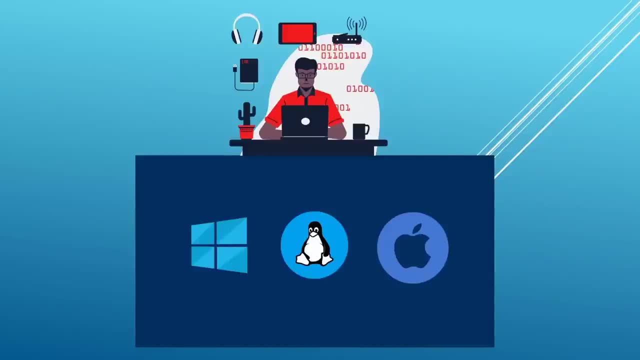 Depending on the operating system you are using to watch the course. If you are on Windows, you're going to install a set of tools that are specific to Windows. If you are on Linux, you're going to install a set of tools for Linux. 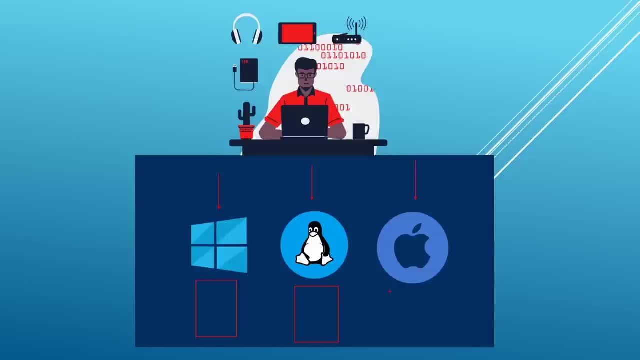 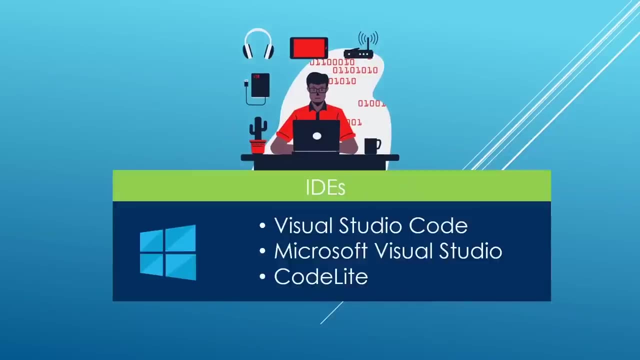 If you are on a Mac, you're going to install a set of tools specific to the Apple operating system for desktop. Now, on Windows, in terms of ideas or integrated development environment, it is possible to use a host of tools. For example, you can use CodeLite. it is an IDE you can use. you can use Microsoft Visual Studio, but in this course, we're going to be using Visual Studio Code because it is easy to install. it has a set of features that are really good. it is popular. it has a great community around it. I think you're going to have a great time, as a beginner, to start writing your C++ programs using Visual Studio Code. 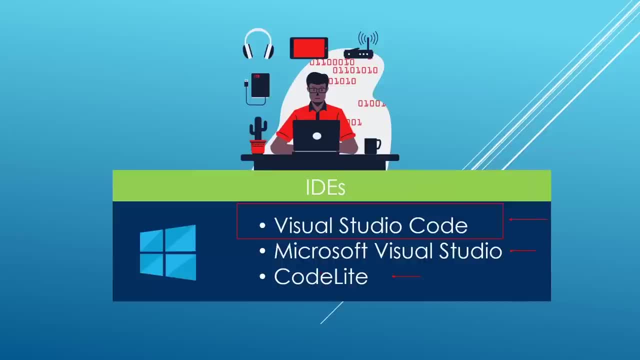 That's not to say that you can't use another IDE. You can If you want, but I am going to be using Visual Studio Code in this course here Now on Linux. we are also going to be using Visual Studio Code as our editor in the course, but there are other ideas you can use. 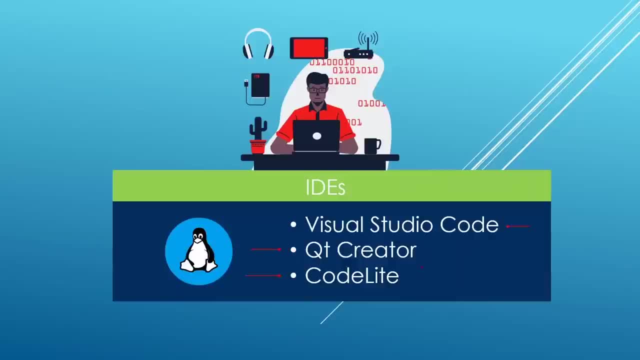 For example, you can use Qt Creator if you want. you can use CodeLite. you can use a host of other ideas on Linux, But again, Visual Studio Code is going to be our thing in the course here and I would recommend installing it on your Linux box if you are watching this course on Linux. 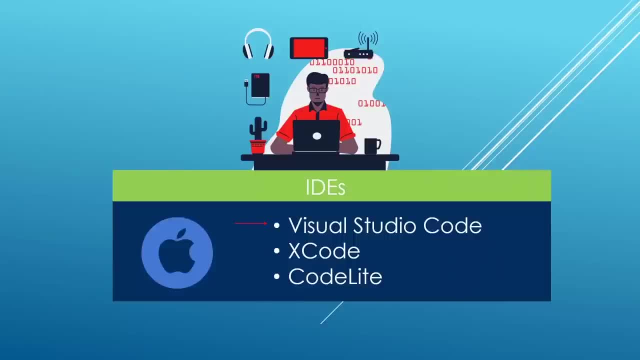 So for OS X, we are also going to be using Visual Studio Code as our editor. As I said, it is cross-platforms. It runs where, regardless of the operating system you might be using, to watch the course. But if you want, you can use the Apple IDE, which is Xcode or even CodeLite. 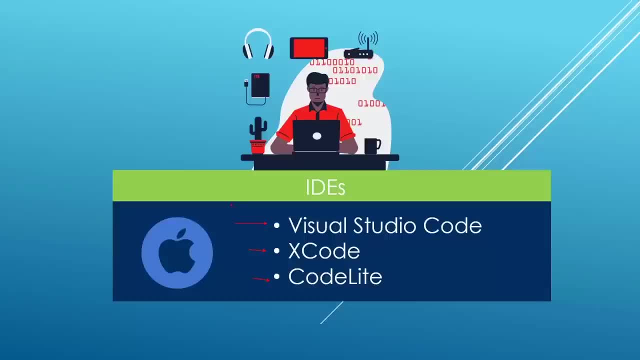 All these are going to work if you want, But again, I would recommend going with Visual Studio Code, at least to start out, so that we have a common ground and you don't get confused very easily, Especially if you are a beginner. Now, after we have an IDE rolling, we will need a compiler. 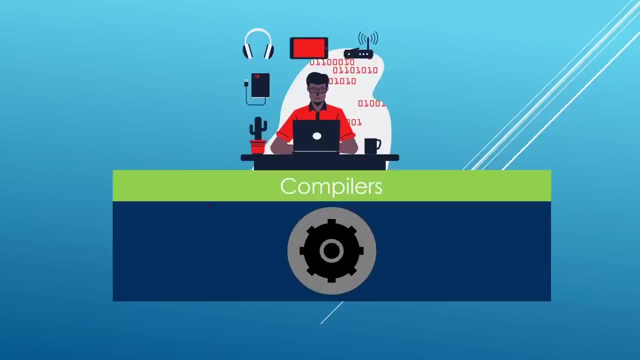 And, as we say, the compiler is a tool that is going to transform your C++ code into a format that can run directly on the hardware. So the compiler you use again is going to depend on the operating system where you are watching the course. 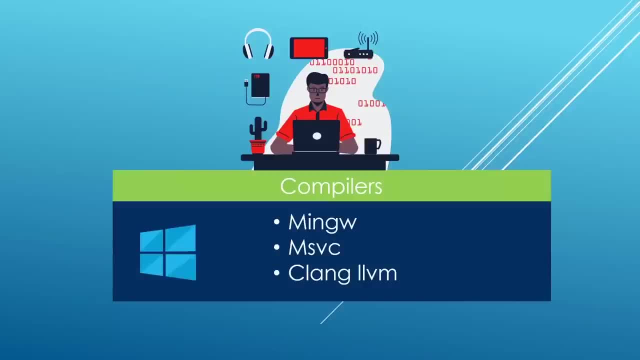 I am going to show you a bunch of compilers you can use, but GCC is going to be our common base. So, on Windows, I will be using what we call the C++. So, on Windows, I will be using what we call the C++. 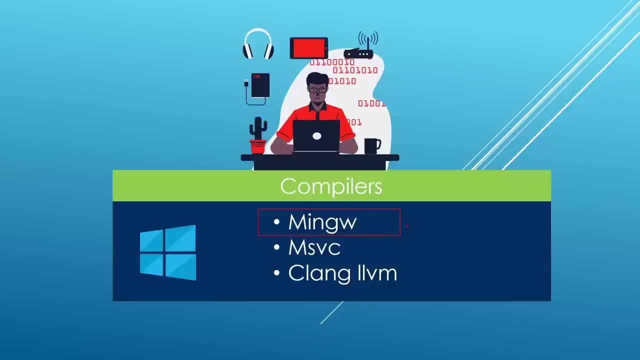 Don't worry, if you don't know what it is, I am going to show you in a minute when we install it. But this is a project that brings the GCC compiler on Windows so that we can use it easily, And I am going to show you how to install it. 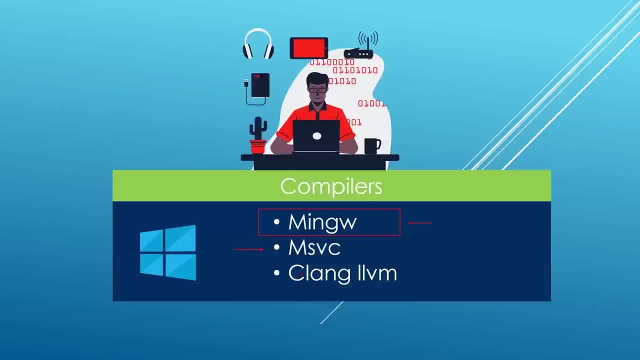 But I am also going to show you how to install the compiler from Microsoft and the Clang LLVM compiler. These are all available to you on Windows And it is really easy to install them these days And I will be using them all. If you are on Windows, I would recommend. 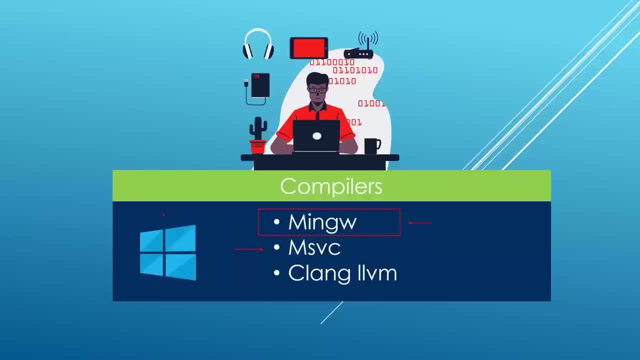 Installing them all so that you really have a chance to try your C++ code on different compilers, And that's a really good thing to do. If you test your C++ code against multiple compilers, you will be increasing your chances for your code to really be portable and work on multiple compilers and operating systems. 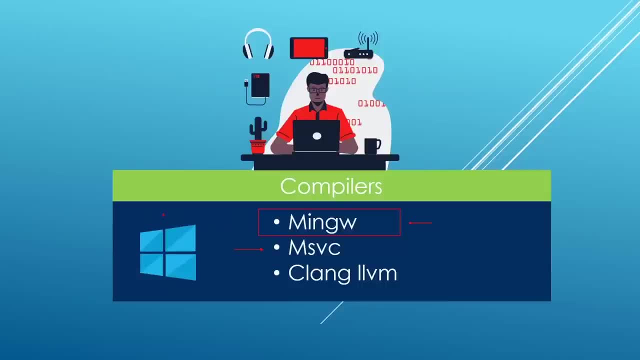 And that cannot be a bad thing. So I would recommend installing all these compilers. if you are on Windows, I am also going to show you how to install two compilers On Linux. I am going to show you GCC. We're going to install the shiny new feature in GCC. 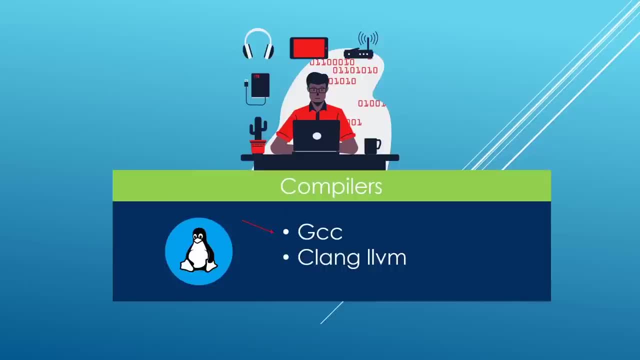 We're going to install Clang LLVM on Linux and we will be able to use all these compilers Again. if you are on Linux, I would recommend installing all these compilers so that you have a chance to try your code against multiple compilers, And that's going to make your code much portable and easier to use on multiple compilers and platforms on the Mac. 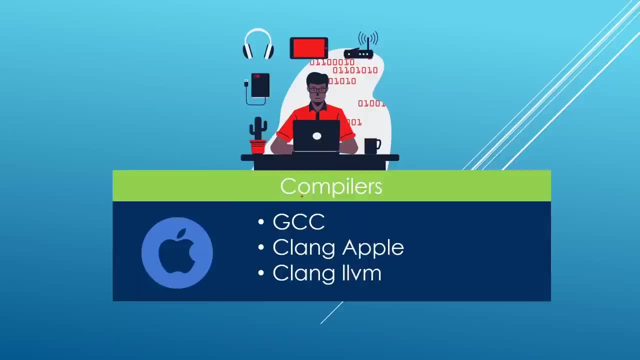 I am going to show you how to install GCC And I am going to show you how to install Clang LLVM. But if you want, you can also install Xcode and the compiler that comes with it for C++ development. All of these are options to you. 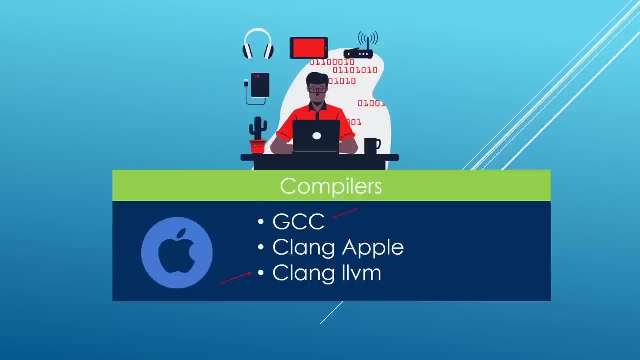 But again, in this course we are mostly going to be using the GCC compilers, So I would recommend getting a hold of this if you don't want to install other compilers. If you only have to install one compiler, please install GCC. That's going to be our main compiler in the course here. 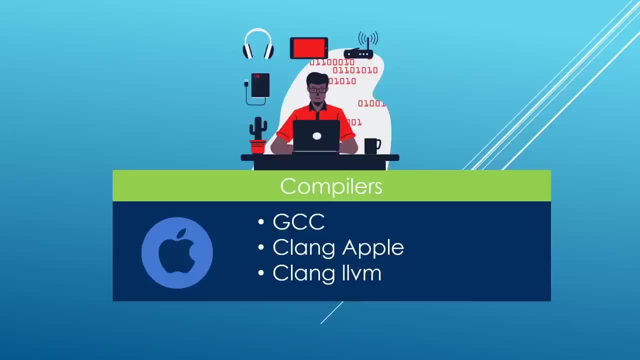 Okay, So these are The tools we need. we are going to head over in the next lecture and show you how to install the Visual Studio Code editor on Windows and really get started with that. Go ahead and finish up here and meet me in the next lecture. 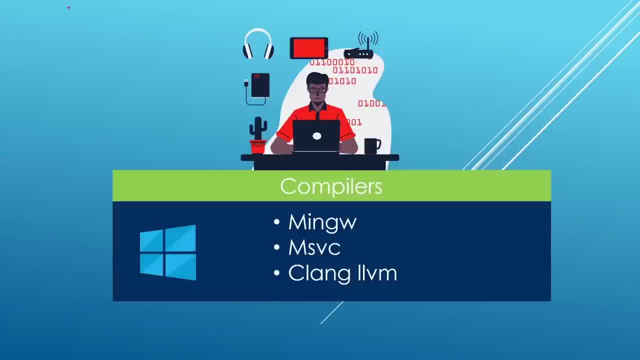 This video I am going to show you how to install a C++ compiler on your Windows operating system. So we're going to be looking at three kinds of compilers. We're going to look at the main GW compiler, which gives us access to a GCC like compiler on Windows. 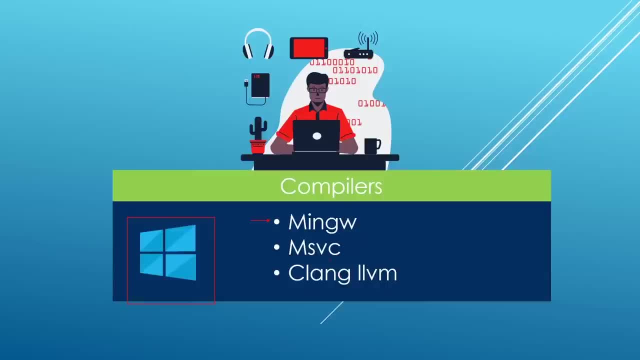 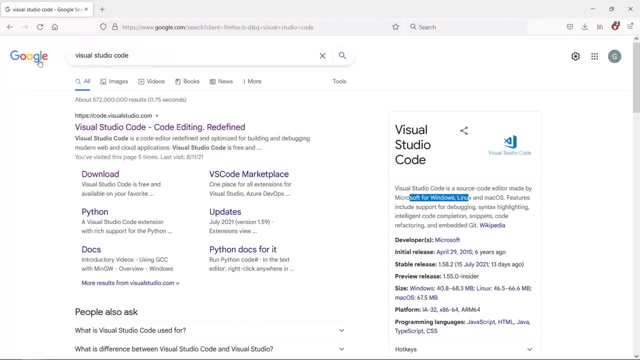 We're going to look at Clang LLVM, which is another compiler. We're going to look at the compiler from Microsoft. Now, before we talk about any compiler, I would like you to come to Google or your favorite search engine and say C++ compiler support. 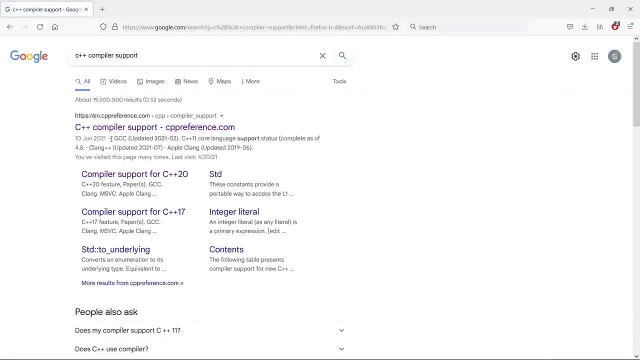 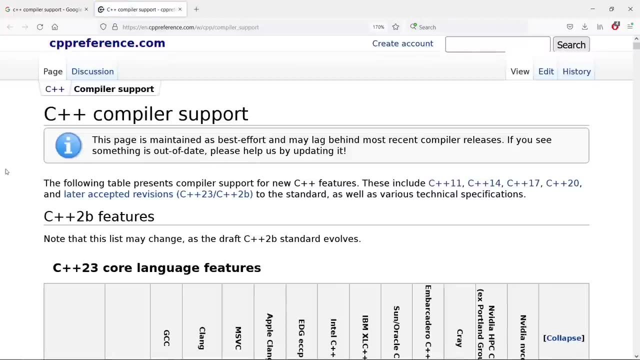 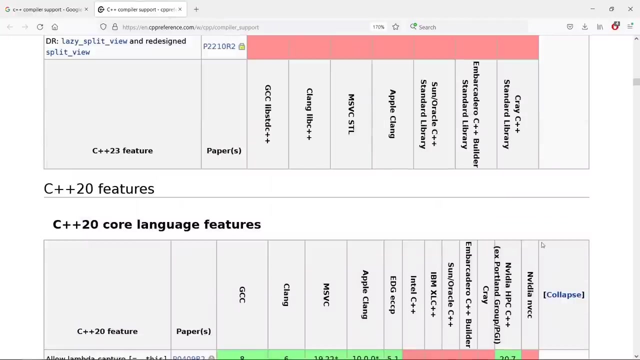 Okay, so we're going to choose this little guy here, And this is really going to give us a bird's eye view on which feature is supported by which C++ compiler, For example, if we are interested in C++ 20,, which is the latest standard that we have in C++ at the time of recording this video. 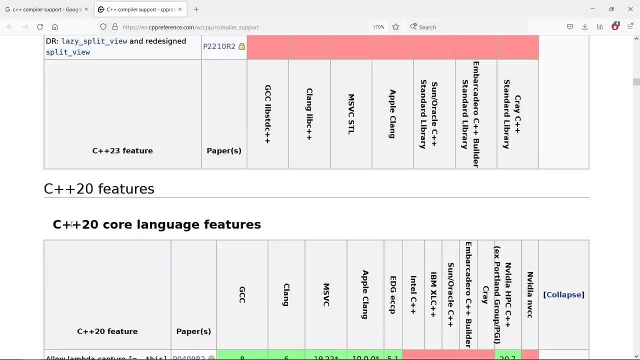 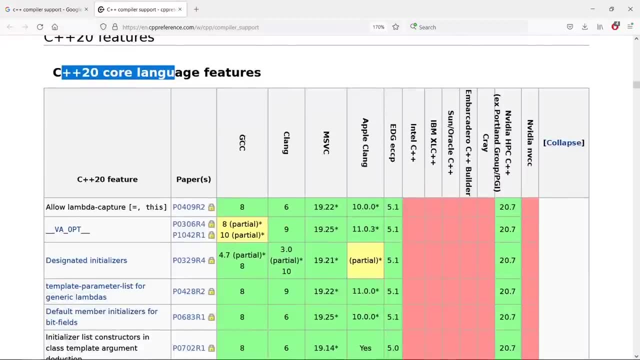 I am recording this in August 2021. But if we go here, we're going to see C++ 20 core features And we're going to see that we have a list of what each compiler supports. We have GCC, we have Clang, we have MSVC. 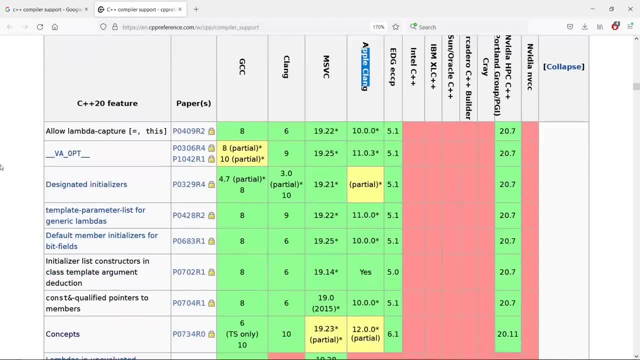 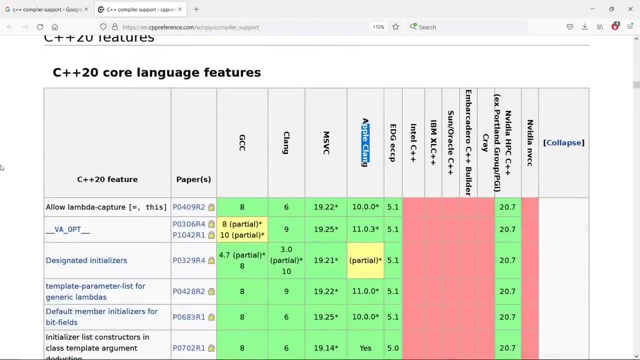 We have the Clang version from the Apple company And if we scroll down we can really see the features that are supported by each compiler. Again, GCC is going to be our choice in this course. This is going to be our main compiler. 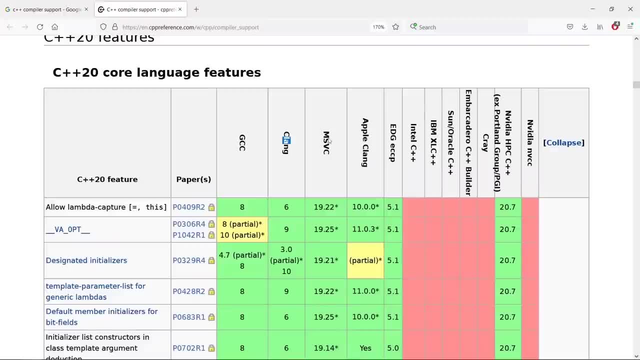 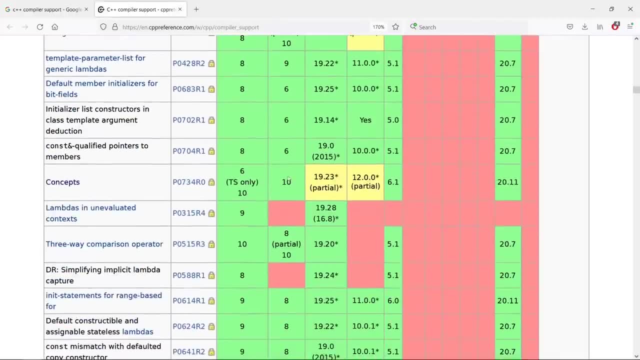 But nothing really stops you from using the Clang compiler or the MSVC compiler, And if you happen to see that your compiler of choice doesn't support what you need, for example, you can see that at the current time, lambdas in an evaluated context are not supported in Clang. 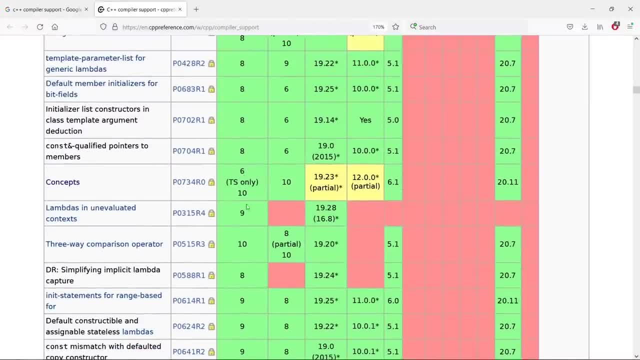 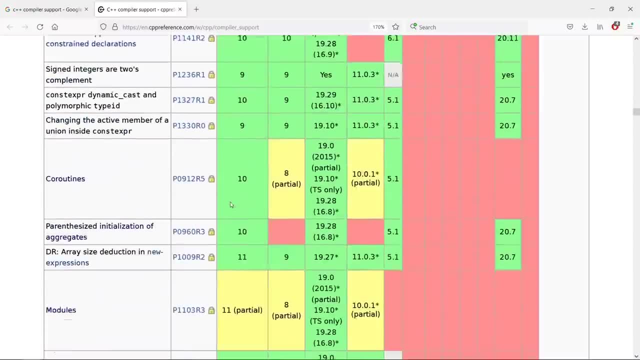 You can see that it is ready here. but this is a feature you can use both in GCC and the MSVC, And this is the MSVC compiler from Microsoft. So keep an eye out on this page here to know which kind of things you can use in your compiler. 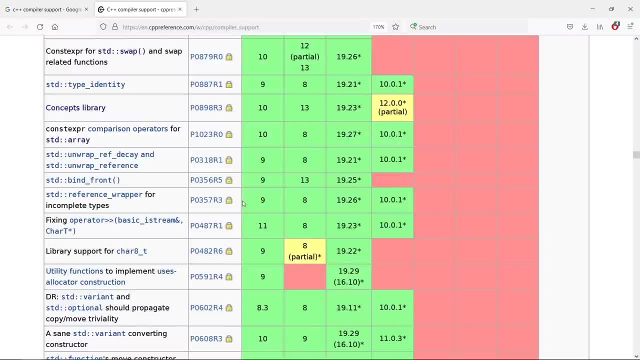 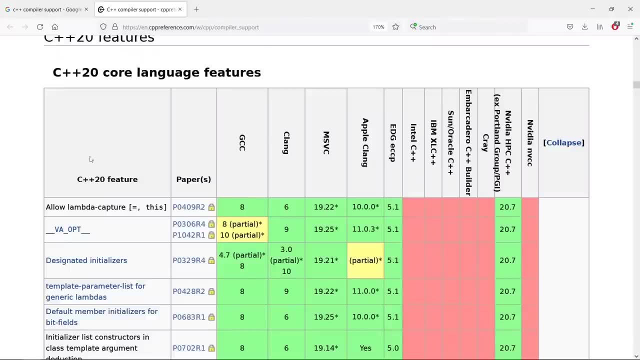 If you try something out and you see that it doesn't work, this is a good place to come and figure out if your compiler supports the feature that you are using. In this video, I am going to show you how to install the three most common compilers. 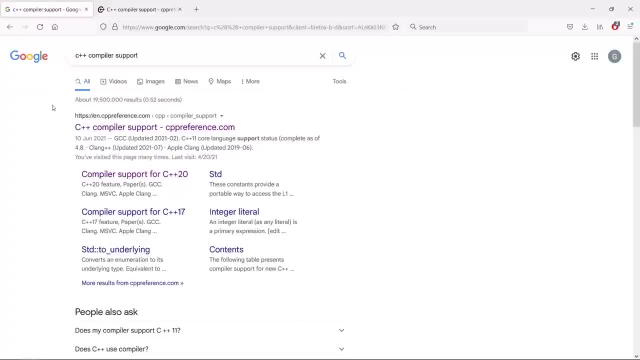 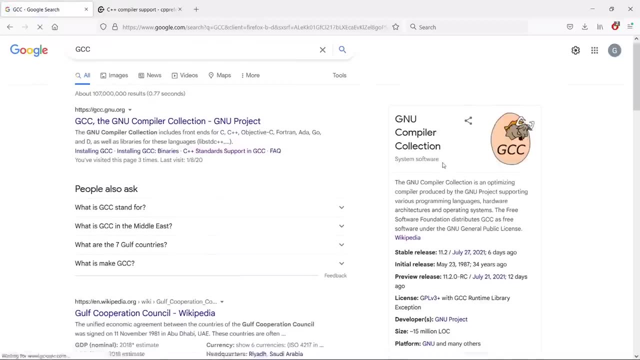 And those are GCC Clang MSVC. If you want, you can come in your search engine and type GCC to see what this is. It is a good thing to do to learn about your tools. here. You can see that it is a compiler that is mostly used on the Linux platform. 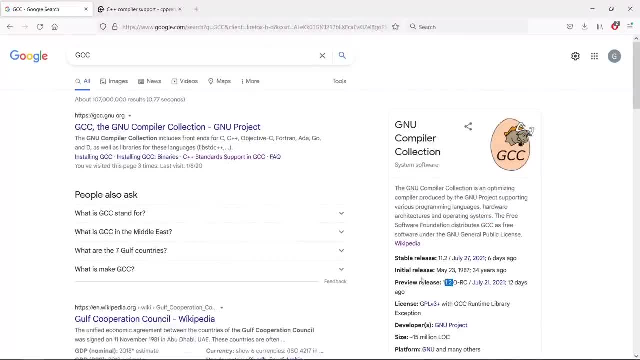 but we can also use it on Windows. The latest release that we're going to be installing is 11.2.0.. I think it was released six days ago, So it is really fresh and we're going to be taking advantage of this. 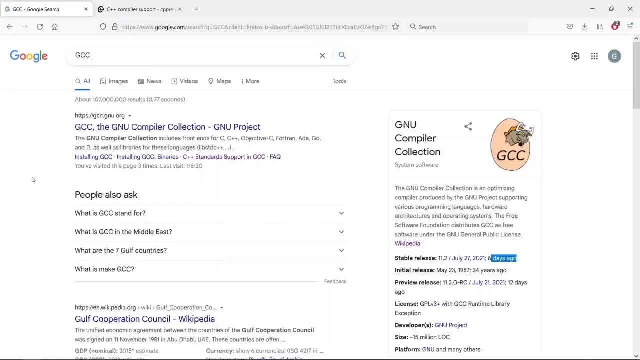 Another thing I should say here is that you should install the latest tools you can get your hands upon. This is the version we're going to be mostly using In this course, But if you are watching this, in the future you're going to have a newer version. 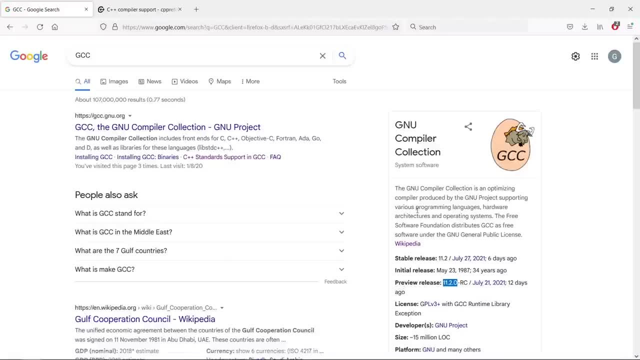 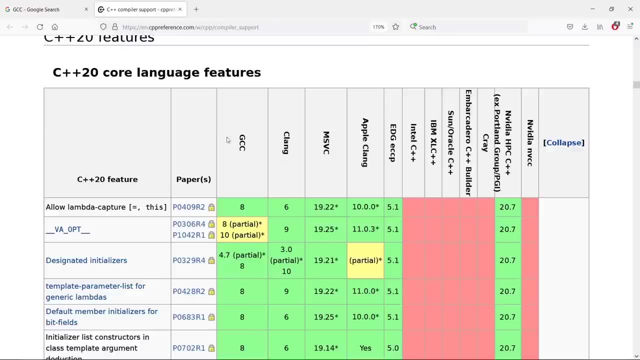 I would recommend installing the latest version or the newest version you can get your hands upon. So the first thing we're going to do is install a GCC compiler on Windows. I am going to show you a way we can get both GCC and Clang in one go. 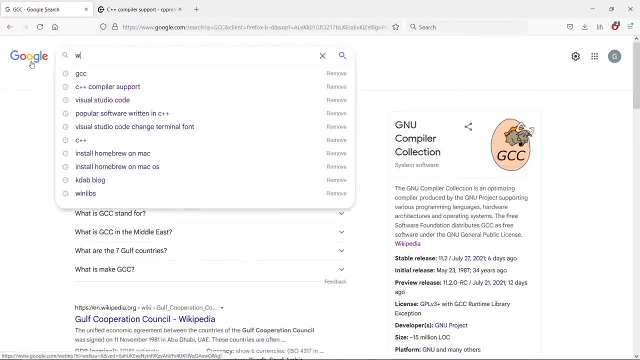 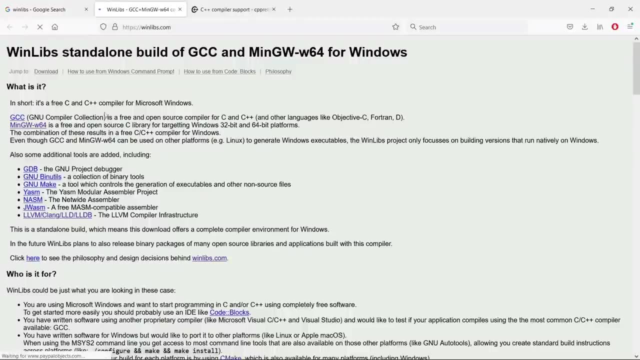 And to get access to that, please go in your search engine and type WinLibs, And this is going to bring us to this project here. If you want, you can click upon this, And this is a cool project by a guy who is providing worlds for these compilers that we can use on Windows. 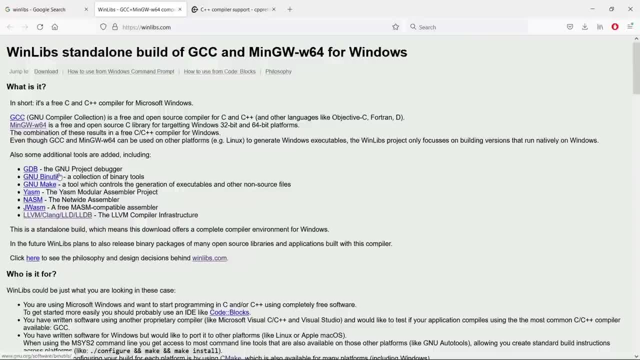 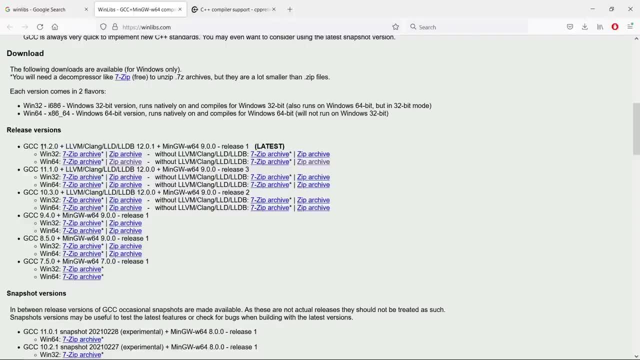 So, if you want, you can just go down here and look at the latest releases. Again, I recommend using the latest you can get your hands upon. In this case, the latest happens to be 11.2.0.. But in the future this is going to change. 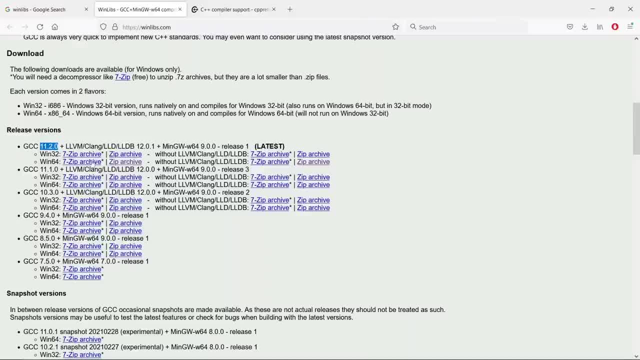 You're going to find a version for 12 or 13.. So please grab the newest version you can get your hands upon. Now I want you to install the version that says that it has LLVM and Clang. So if you are on a 32-bit version on Windows, I would recommend getting this 7-zip archive or this zip archive here. 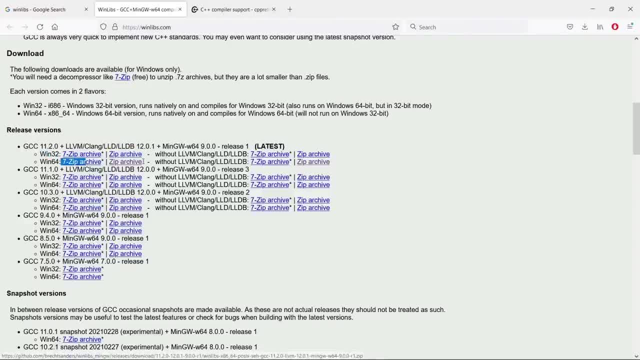 If you are on 64, I would recommend getting a hold of this or this little thing here. It doesn't really matter, But make sure you get the latest version you can get your hands upon, And you can see that this conveniently says latest here. 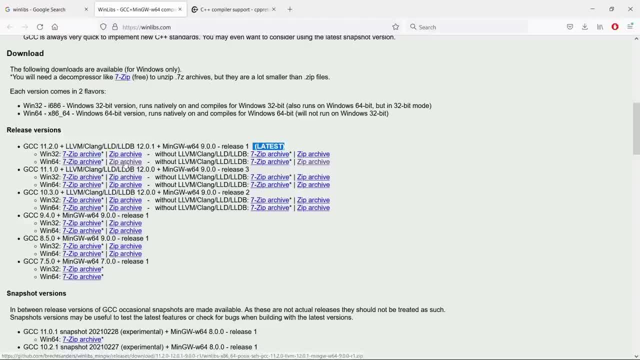 So I am going to download the 64-bit version On Windows. I am going to grab the zip archive here and let's click upon this. This should kick off my download and this is going to download on my system. I can download this if I want. 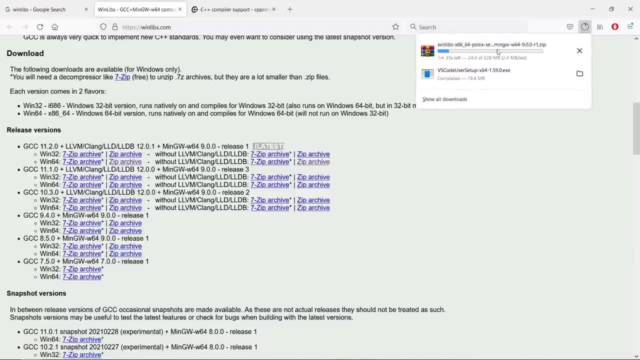 And you're going to see that it is going to start downloading here And I am going to wait for this to finish. Again, this is going to give us both the GCC compiler and the Clang compiler, And this is really like shooting two birds with one stone. 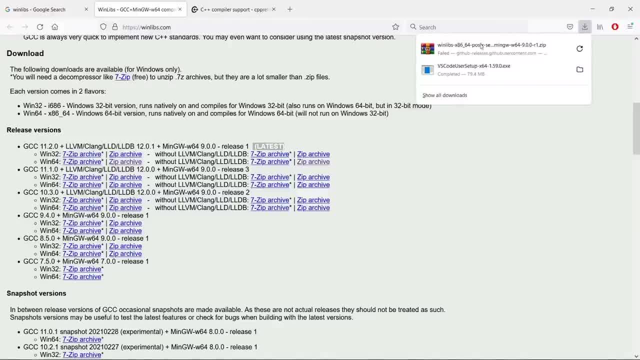 So this is going to be really good. I already have This downloaded, So I am just going to head over to the location where I have this downloaded. I think I can just go in my drive here. So let's crack this open and go in my downloads folder. 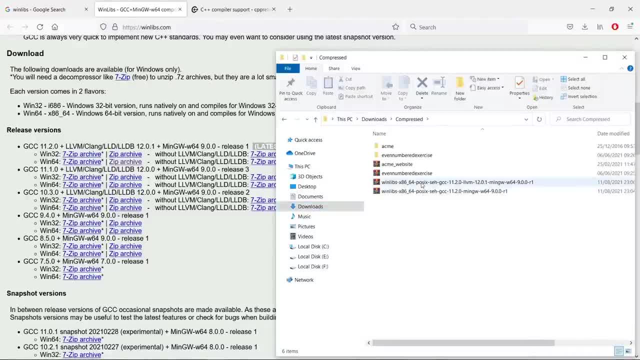 And if I go in my compressed folder, I am going to find Winlabs, LLVM and MinGW. This is what you really want. But if you don't want the Clang compiler, you can grab the one that doesn't say LLVM here, because we really want both of. 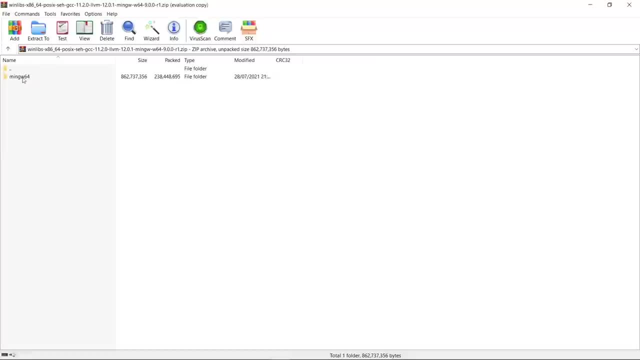 These compilers. We are going to grab the one that has both of the GCC compiler and the Clang compiler. If we crack this open, let's open this together so that you can see what is happening. We are going to have this little folder here. 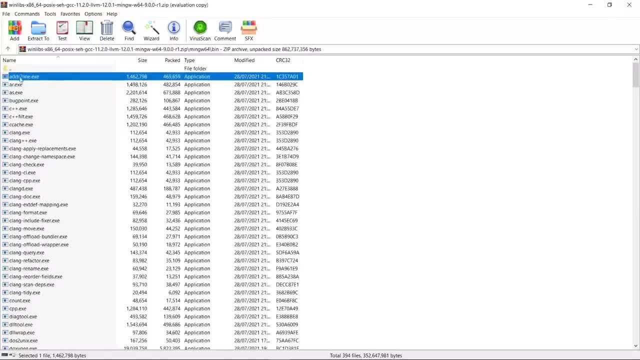 If we go in, we're going to find a bin folder. If we go in and crack that open, we're going to have a folder that says Clang. You see, we have our Clang compiler. We have our Clang++ compiler for C++. 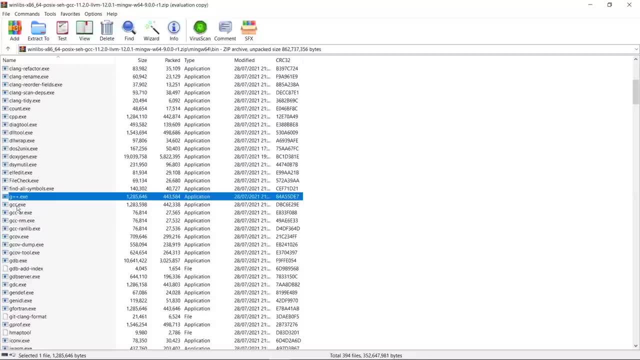 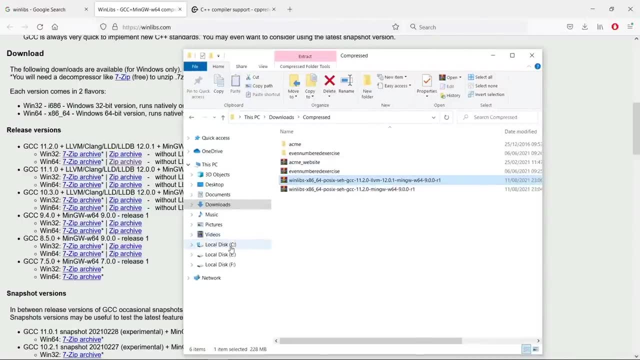 And if we go down, we're going to find our G++ compiler And the GCC compiler. This is what we want. So what we are going to do is extract this somewhere on our system. I put this on my C drive, So if you go here, you're going to find MinGW64.. 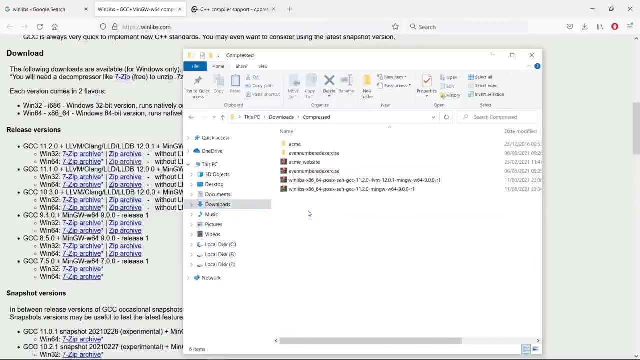 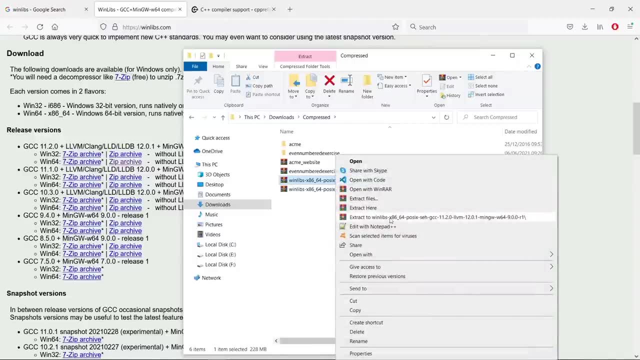 So all you really have to do is go where you downloaded your compiler and say extract. We're going to right click on this and say extract to a location, and you're going to specify where you want this to go And this is going to be extracted. 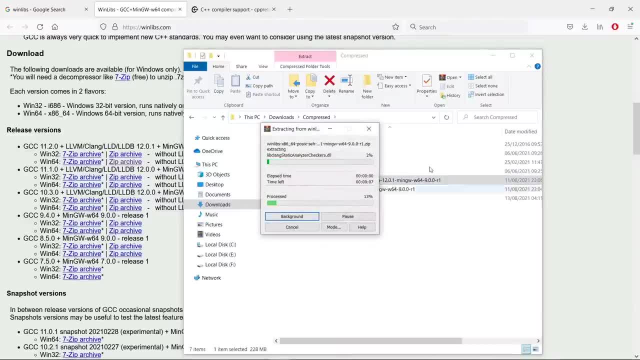 Or even, if you want, you can extract here. This is something I like to do. This is going to show up in the current folder and you can grab this and paste that in a location where you want this. In my case, I put this in my C drive, as I said here. 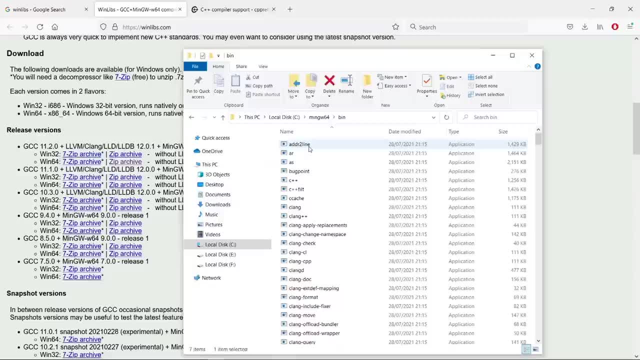 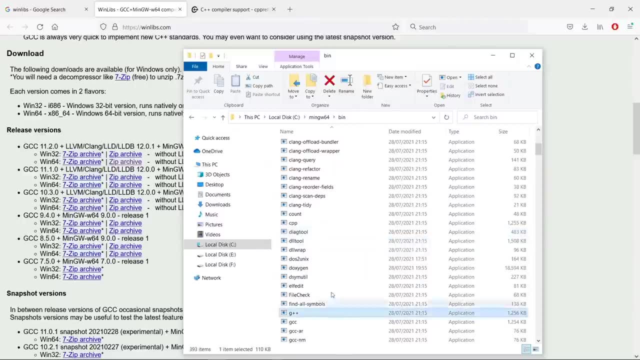 So this is going to be my compiler. Now, once you have these compilers installed again, we have the Clang compiler, We have the GCC compiler. If we go down, we're going to find the G++. We even have GDB, which is a debugger we can use to debug C++ applications. 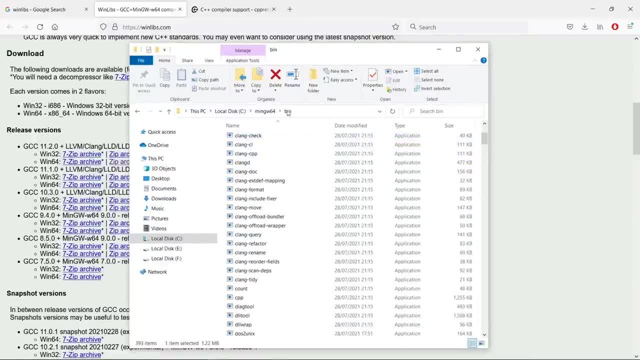 But we will talk about this later. But before we have this, I would recommend putting this in your environment variables on Windows. The way you do this, you grab this path. Well, we have our compilers here and we're going to copy this. 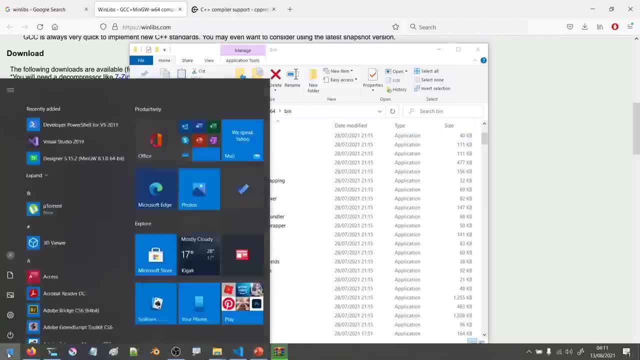 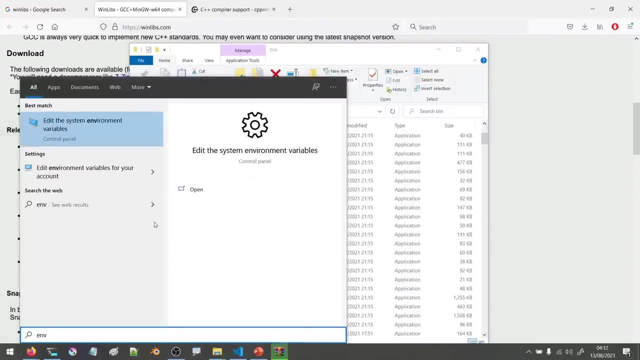 This is something I recommend, And on Windows 10, you can go on the start menu and type env, And this is going to give us a window in which we can edit our environment variables. We're going to click on this little thing. 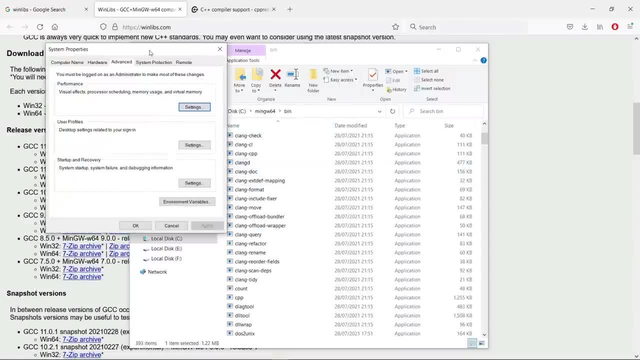 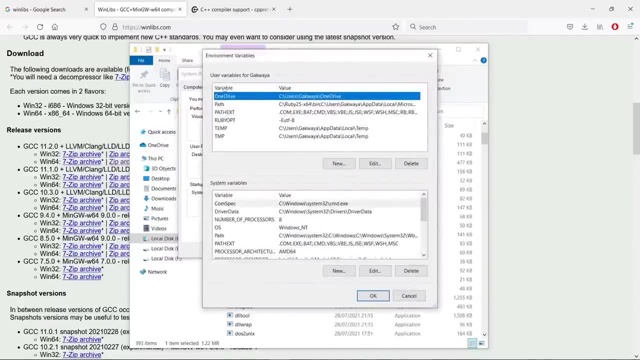 This is going to open up on our system. We're going to wait for this to open up. We're going to have a window that says system properties. We're going to click on environment variables here And we can put this in our user environment variables or on our system environment variables. 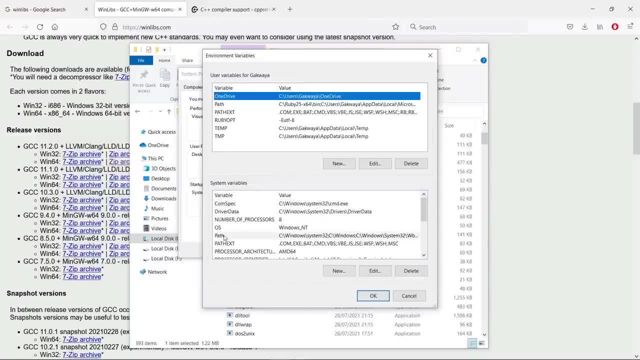 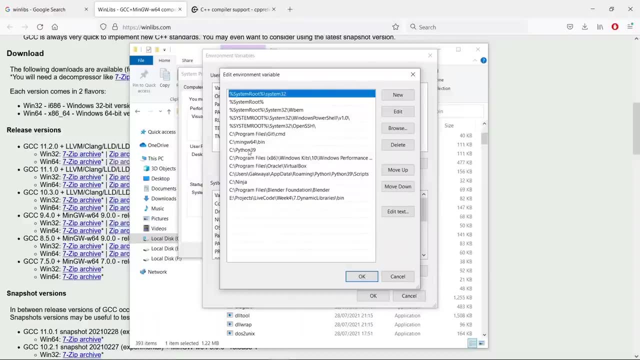 Since I am the only one using this system, I like to put this in my path for my system variables. So I am going to click on path and click edit here, And I am going to add a path to my GCC and Clang installation here. 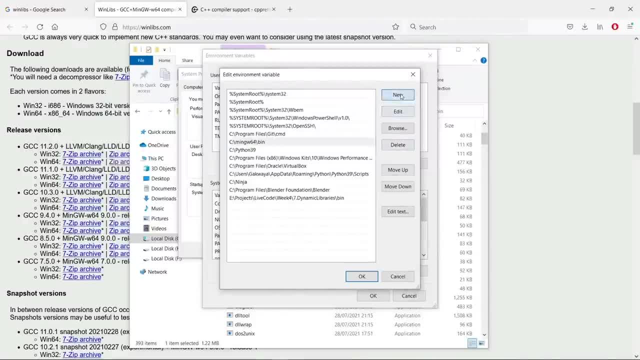 You can see that right here. If you don't have this end, you can Click on new. You're going to have a window here and you can paste this right in and you can click Okay, but I'm not going to do that because I already have this in here. 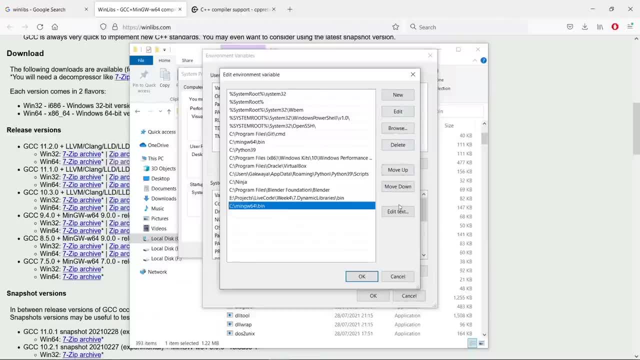 So what I am going to do is just delete this. Let's see if I can delete. I can delete this little guy and I have my path in here. So if you don't have this end, please make sure you have this in your environment variables. 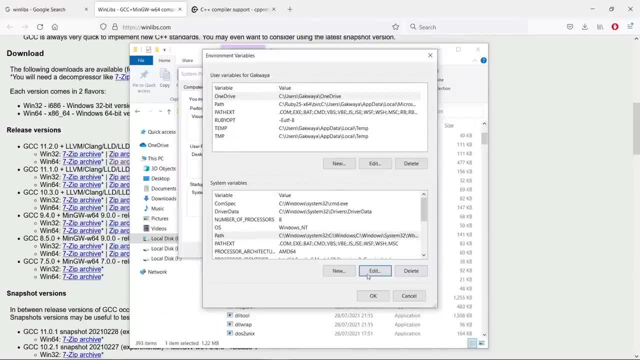 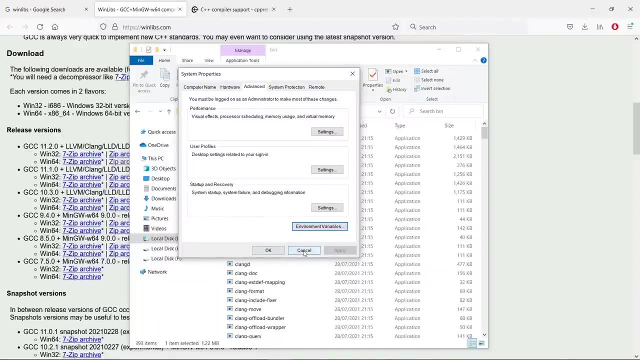 So we're going to cancel out of this. But if this is the first time you do this, you should click Okay. And one way to test That your environment variables are working, or even if your compilers are working, is to crack up a command line terminal. 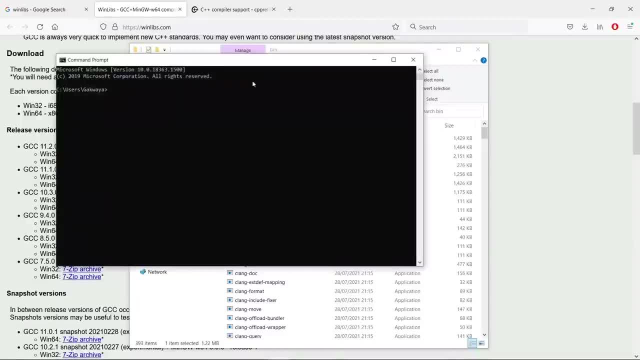 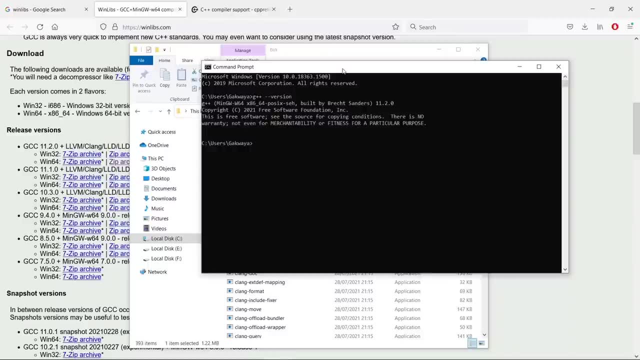 So we're going to say cmd on the start menu here, And all you need to do is say G++, just like this dash, dash version. If you do this, you're going to see information about your C++ compiler, And this is coming from the installation. 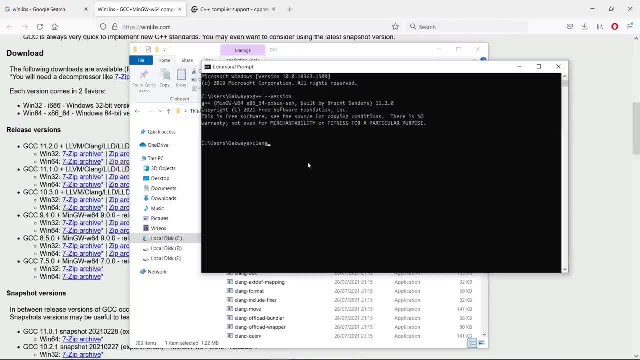 We just did, and for Clang you can say Clang++ version And this is going to tell you the information about your Clang compiler installation. Let's wait for this to come up. I don't know why it's slow, but you can see that we have our Clang compiler. 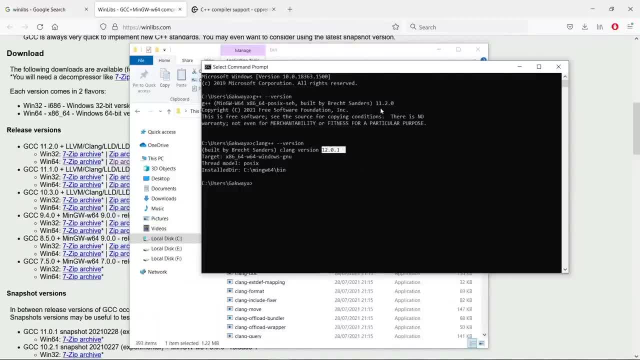 The latest version is 1201. for the GCC compiler, The latest version is 1120.. And these are the compilers we can use to write C++ 20 applications. Okay, So by now we have a GCC compiler through the main GW project. 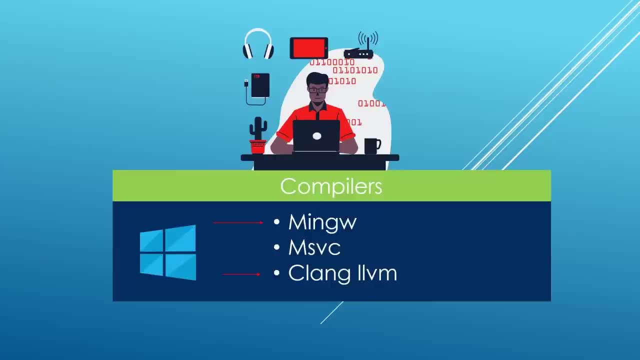 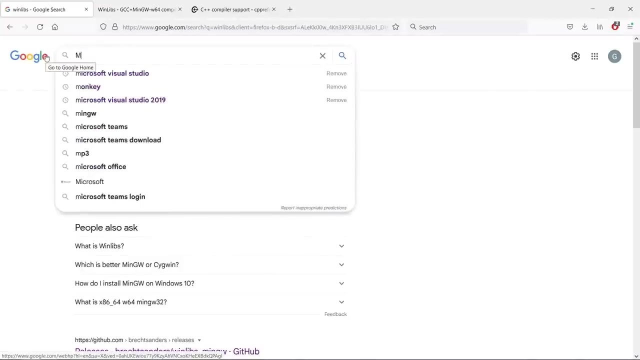 We have a Clang LLVM compiler on our system. We are also going to see how to get a hold of the compiler from Microsoft. And to get a hold of this, you need to install Microsoft Visual Studio. To install Microsoft Visual Studio, all you have to do is come to your favorite search engine and say Microsoft Visual Studio. 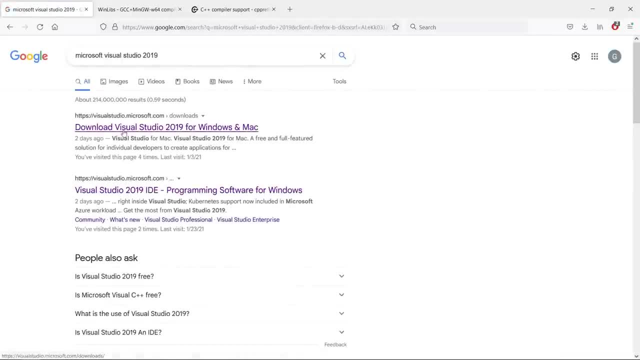 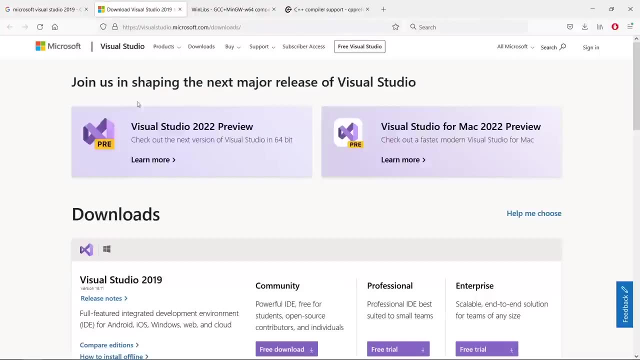 We can look at the 2019 version, which is the latest, I think, And we're going to click on the download link here we have as the first link And we're going to see ways we can download this little guy Now. 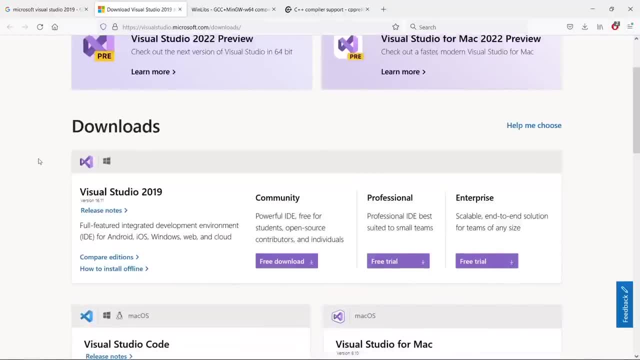 Microsoft Visual Studio has a community version you can download for free, But we also have a professional and Enterprise versions that we're not going to care about in this course. here We are just going to download the community version, and that's going to be enough for our purposes here. 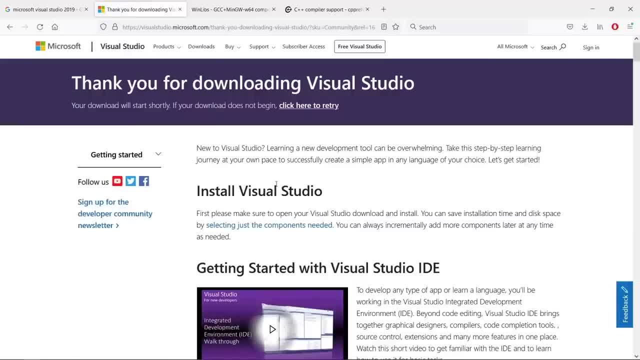 So if you click on free download here, this is going to download and install the Visual Studio compiler. You can click on this little guy and it is going to download an installer. You're going to crack this open on your system And it is. 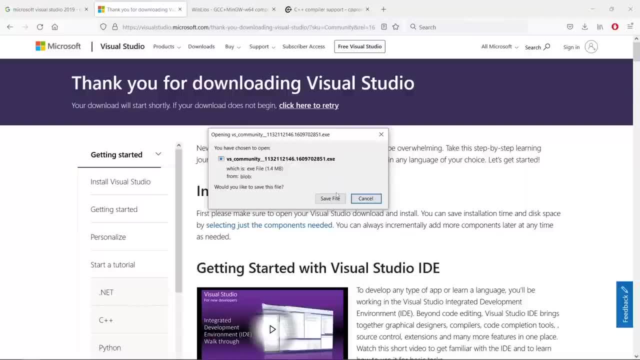 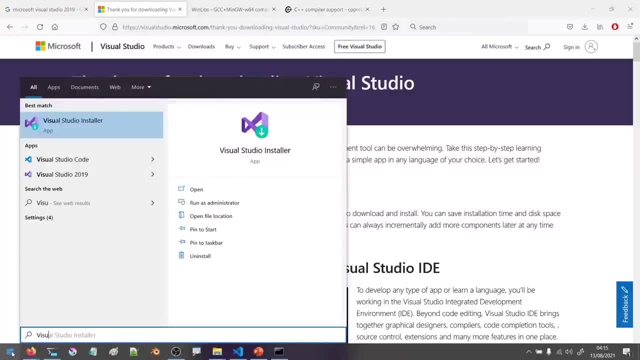 And it is going to install the Visual Studio installer. So once you have it installed you can come to the Start menu here and say Visual Studio installer. I think If you say Visual Studio you're going to have this pop up somewhere on your system. 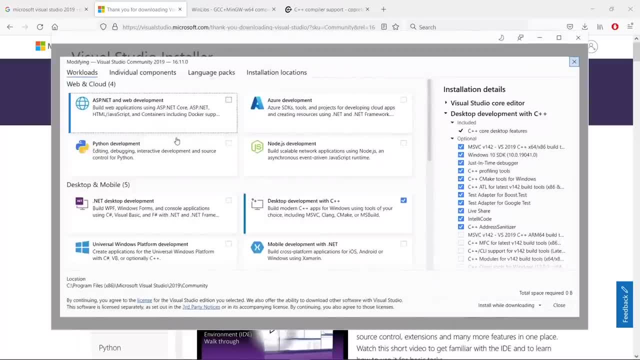 We're going to click on this And if you crack the installer open, you're going to see a window like this, which is really going to give you a chance to install the tools you want to use with the Microsoft Visual Studio IDE, And in this case, we are interested. 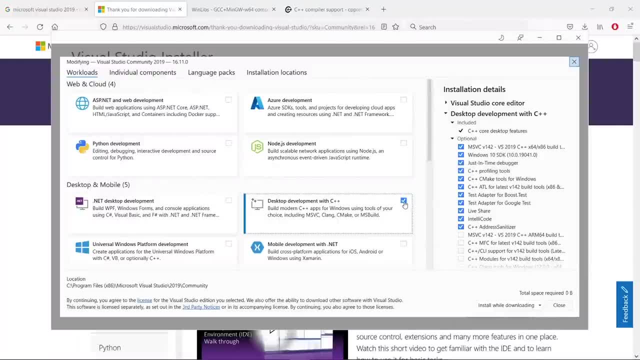 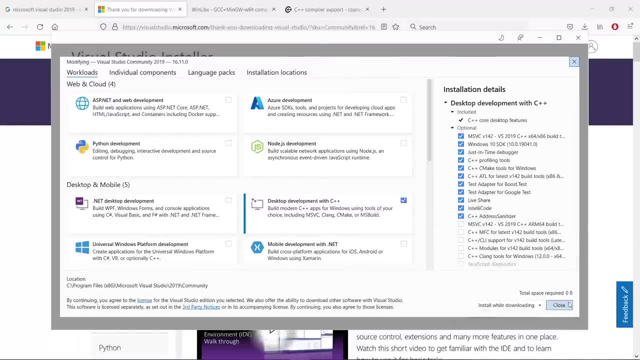 In desktop development with C++. So we're going to click this little guy here, We're going to take it open And once you do this, you going to click download and install. And this is going to install the Visual Studio compiler with the underlying compiler. 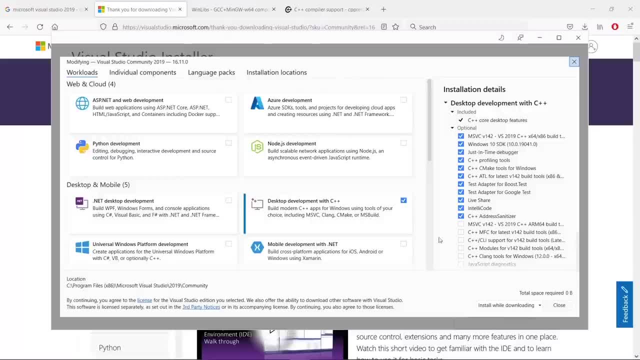 You see that this is going to give us access to the MSVC compiler and all kinds of crazy things. We really need it to write C++ applications on Windows using the compiler from Microsoft. Now I have to say this is going to take some time to install. 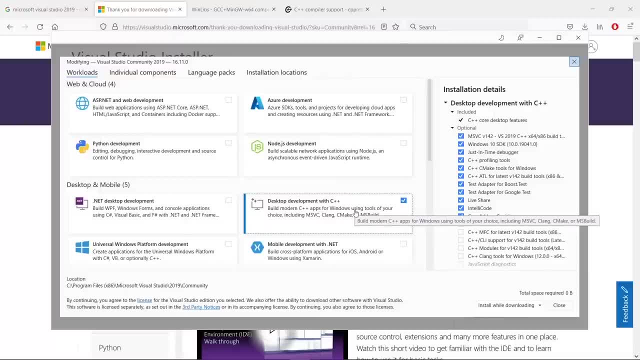 So if you see that this takes up 20 minutes of your time, don't worry. This is really normal, because this IDE and the compiler behind it are really large. They're not like the GCC or the Clang LLVM compilers that we just installed. 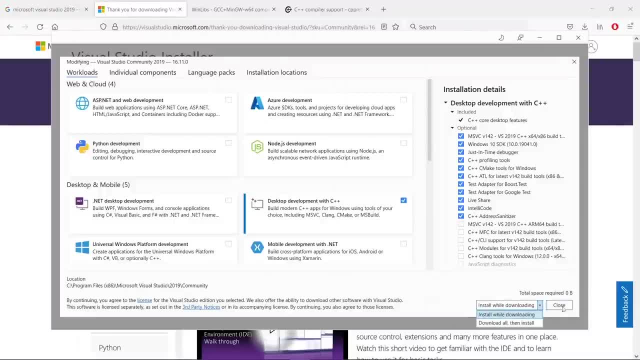 OK, so once you have this ticked or checked, you're going to click on download or install whatever this button is saying here. This is going to install both the Microsoft Visual Studio IDE and the compiler from Microsoft that you can use directly To write C++ applications. 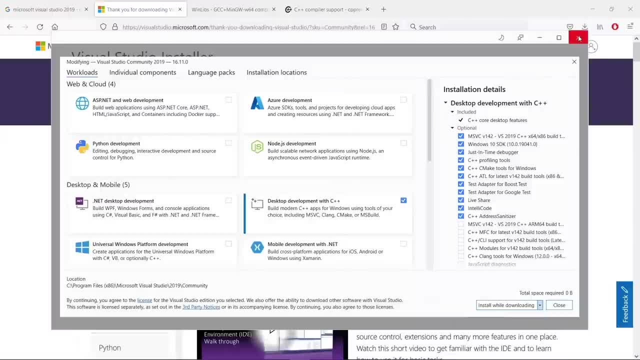 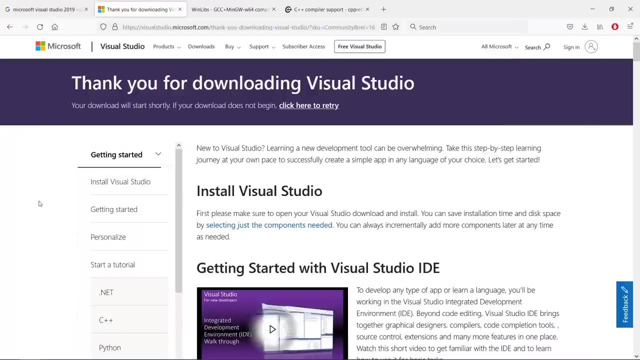 So once we have this open- I am going to suppose that you have this installed already- I am going to close out of this because I don't want to do this- And you're going to have Visual Studio installed on your system. Once you have this installed, you're going to come to the start menu and say developer. 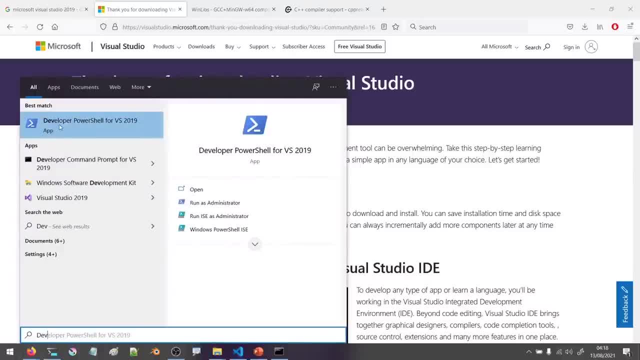 And this is going to bring up two things. One is going to be the developer PowerShell for Visual Studio 2019.. And the other is going to be a command prompt. It doesn't really matter what you choose. I am going to click on command prompt. 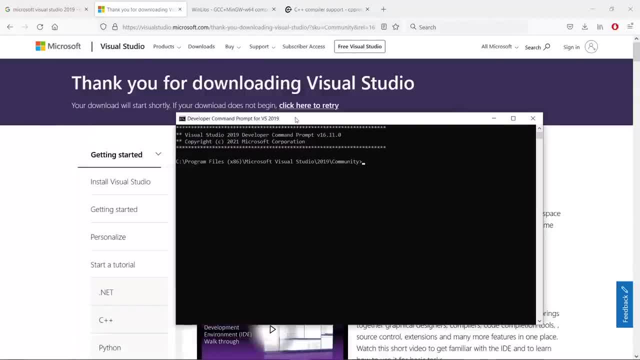 And once you do this, this is going to give you a terminal or a window through which the environment variables are already in, to start using the compiler from Microsoft. And if we come here and type clexe, we're going to see that. We're going to see the information here. 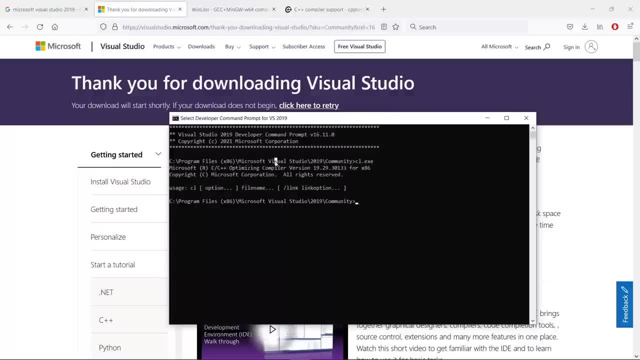 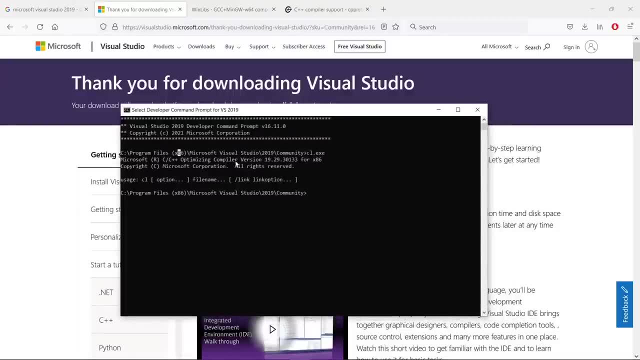 If this gives you an error or something, you're going to know that you didn't really install this properly. So please go back and make sure you have this installed. If you have a problem, you can ask me. I can do the best I can to help you out. 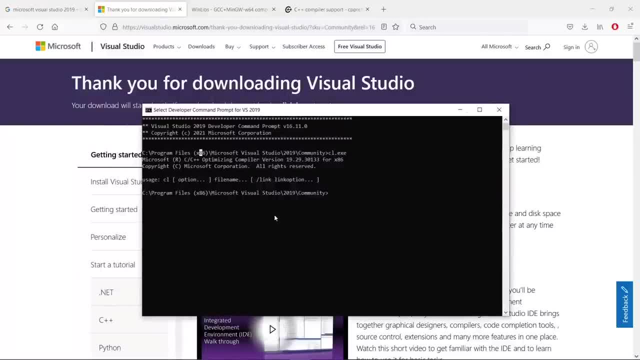 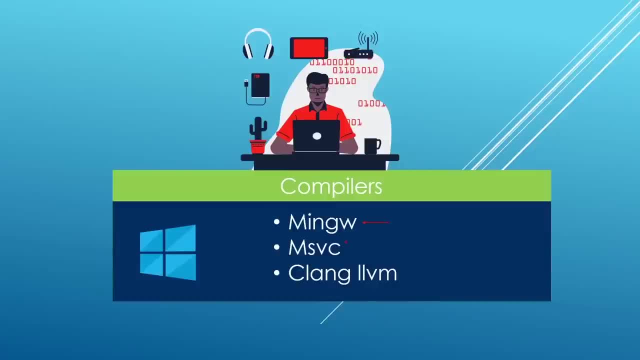 But by this moment we have three compilers on Windows that we can use for C++ development. We have the MinGW or the GCC compiler in our hands, We have the Clang LLVM compiler And we have the compiler from Microsoft, And now we can install an IDE or an editor. 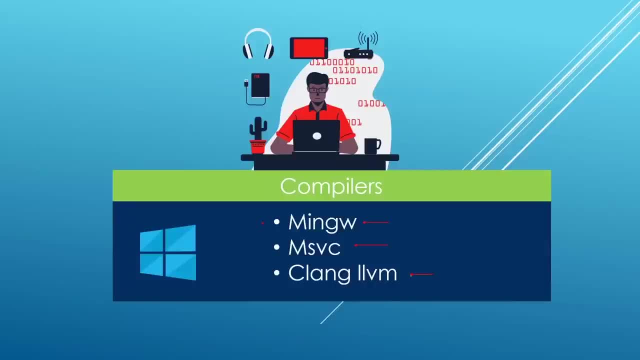 And that's going to be Visual Studio Code And we can connect that to this compiler so that we can start writing our own C++ 20 application. We are going to head over in the next lecture and install the Visual Studio Code editor. Go ahead and finish up here and meet me there. 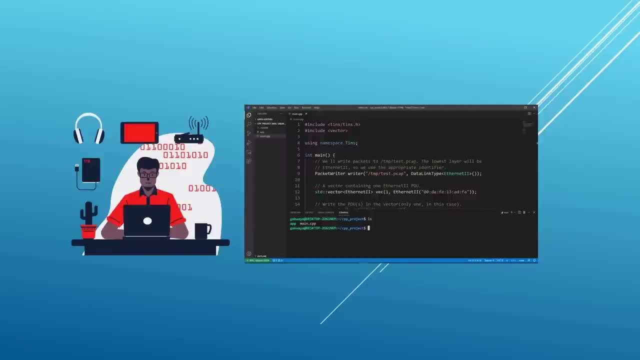 In this lecture I am going to show you how to install the Visual Studio Code editor on Windows. So if you are watching this course on Windows, this video here is going to be a must watch. We are going to head over to our search engine and type Visual Studio Code. 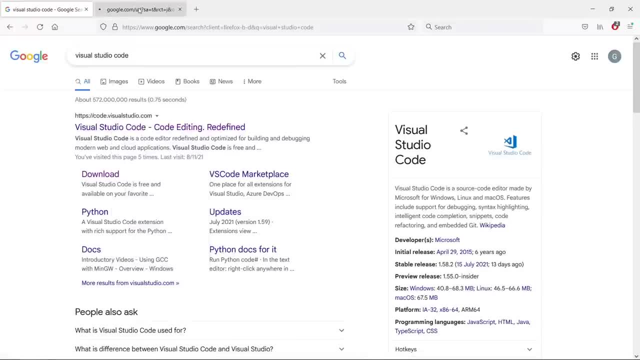 This is going to give you a link where we can download this cool editor If you want. you can learn all you can about it. It is a source code editor made by Microsoft. It supports multiple languages, But we are going to be using that specifically for C++ in the course here. 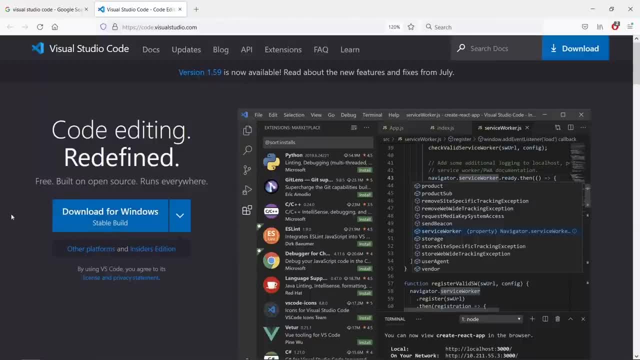 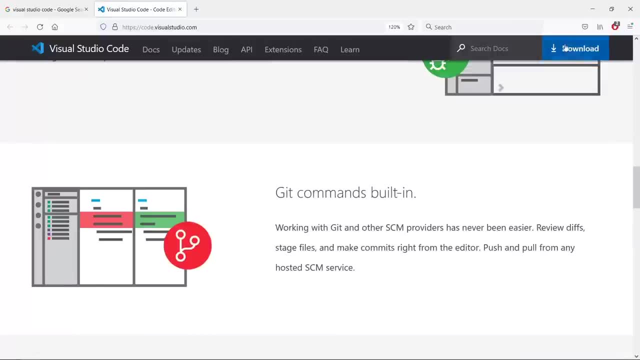 Here I am at the page for the editor And you can read all you want about it. But we are interested in downloading this for Windows. If you want, you can click on this download button here, But I am just going to scroll down and have download links for Windows. 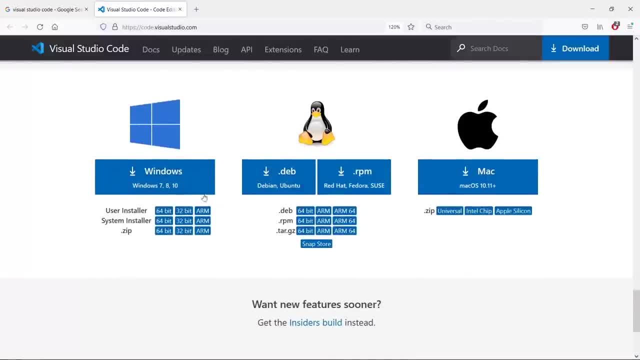 If I want, I can click on user installer- system installer. You can click on what you want. If you are on a 32-bit system, you are going to download a 32-bit version. I am just going to click on 64-bit here because I am on a 64-bit operating system. 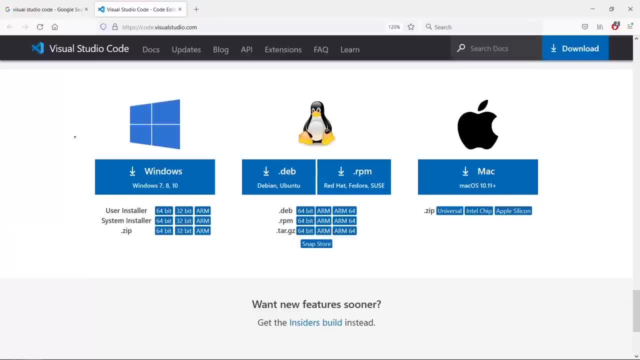 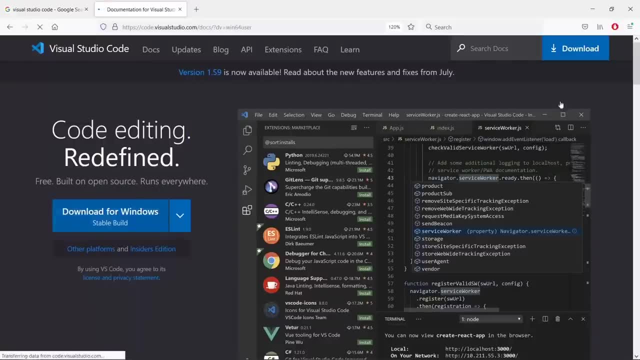 Again in this video. we are doing this for Windows, So this is going to be our area of interest here. I am going to click on this download link And I am going to wait for things to kick off And I will have a window to start. 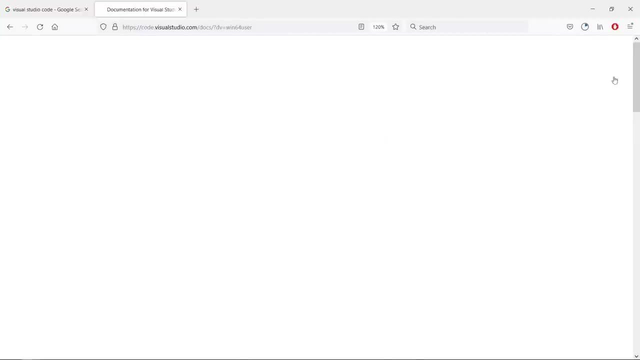 Downloading Visual Studio Code setup. here I can save this file and it is going to start downloading Once it is downloaded. I am going to double click and really click my way through this until I have Visual Studio Code installed on my computer here. 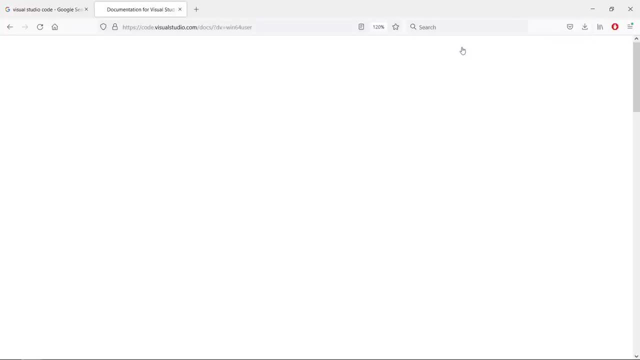 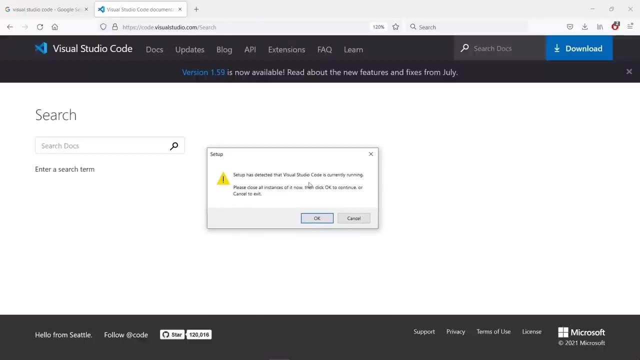 Okay, the download is good. I can crack this open. Let's click on this And you are going to see that it is saying that it has detected that Visual Studio Code is already running on my system, because I have it installed. But if you don't have it installed, 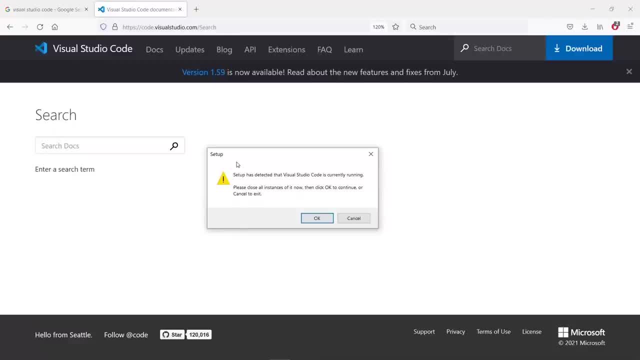 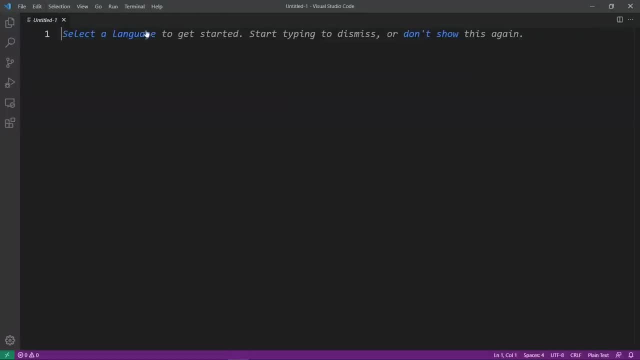 you are going to click your way through and install this on Windows And after you have it you can start it. Okay, once you start Visual Studio Code, you are going to have a window like this: If you run it for the first time, you are probably going to see a Windows with documentation and whatever. 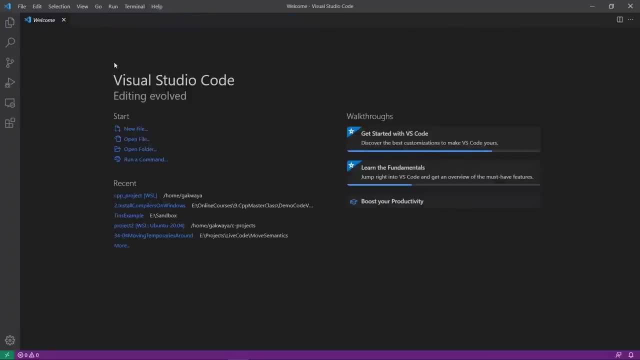 Let's look at the welcome screen. You are going to probably see something like this, but I am not sure. But the most important thing is that you are going to have a window like this with Visual Studio Code. So what we want to do for C++ development is going to scroll down and click on this little thing that says extensions. 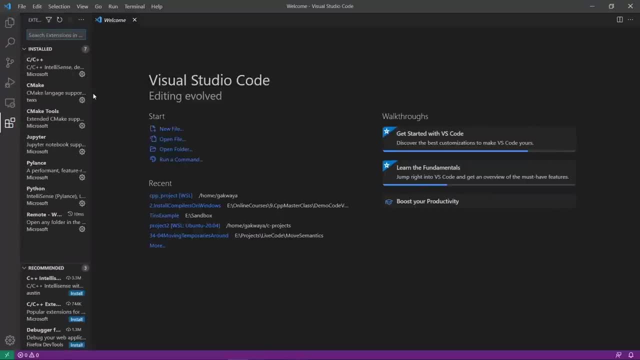 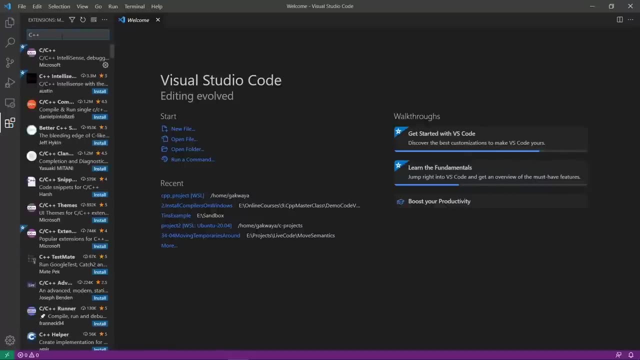 I am going to click on this and I am going to go in my search box here and type C and C++. I can even type C++, It doesn't really matter- And this is an area where we can install extensions to make Visual Studio Code do all kinds of crazy things. 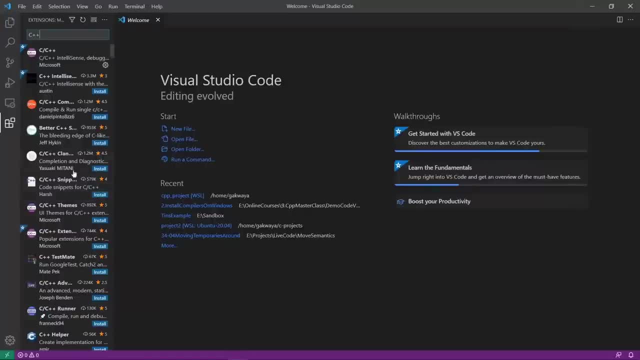 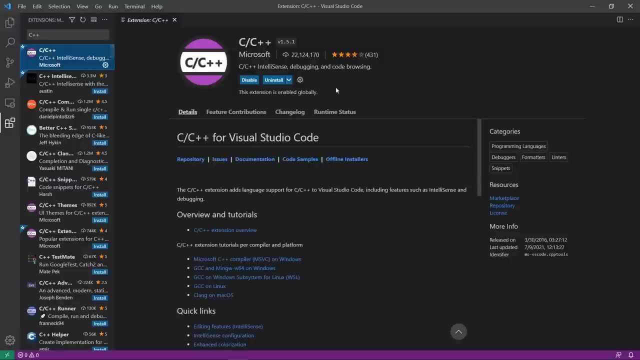 In this case, we are interested in making it support C and C++, So we are going to click on this extension that says Microsoft here, C and C++. I am going to click on this And if you don't have it installed, you can click on the install button. 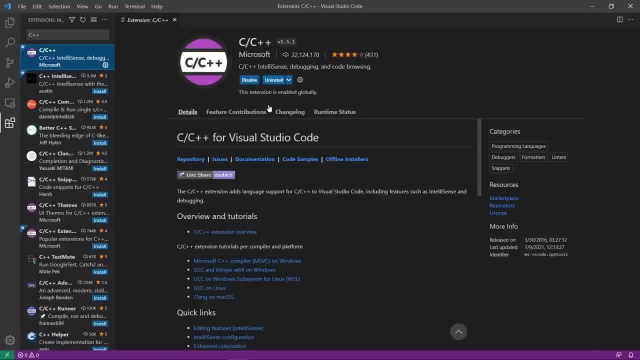 And it is going to install this little thing and make your computer ready to use Visual Studio Code for C++. So make sure you install this And at the end it is going to say disable or uninstall, because it will be already installed and enabled on your computer. 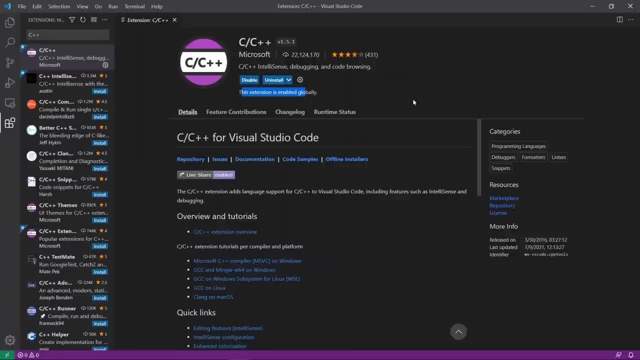 And this is really the end. This is the end of our installation video for Visual Studio Code. We are going to head over in the next video and show you how you can make Visual Studio Code use the compilers that we installed in the previous video. 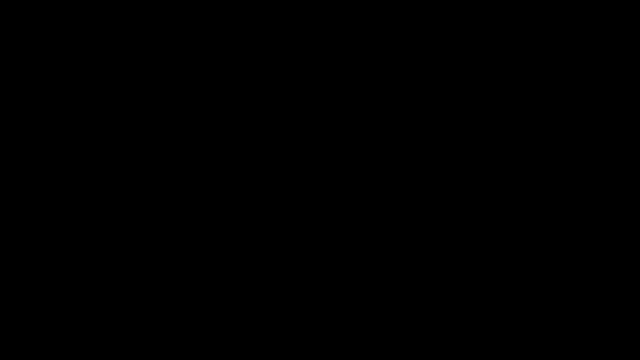 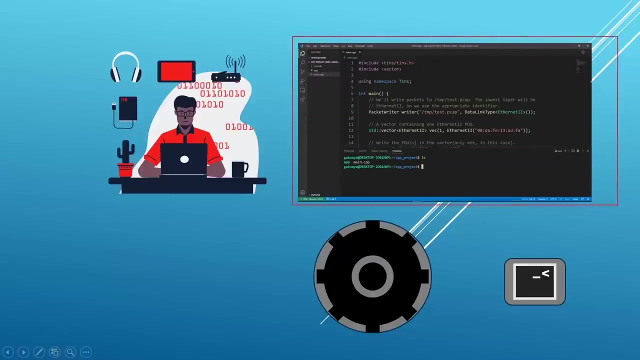 So go ahead and finish up here and meet me in the next lecture. In this video, we are going to see how to connect our Visual Studio Code editor to a compiler so that we can compile our project easily through the Visual Studio Code editor. We already have the IDE installed. 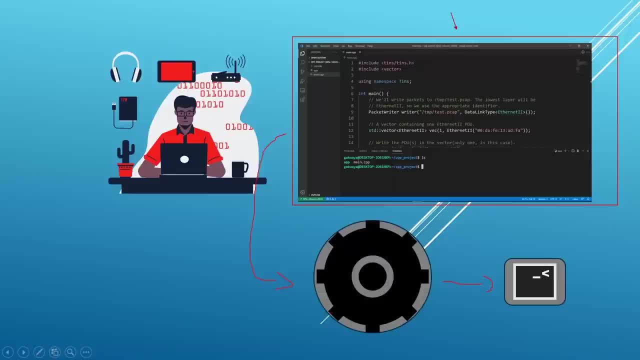 From the last two previous lectures- when we have a compiler installed. In the last lecture we installed the GCC compiler through the main GW project. We installed the Clang LLVM compiler. We even installed the compiler from Microsoft. Now we are going to connect the IDE to the compiler to make it really easy to compile C++ applications using these tools here. 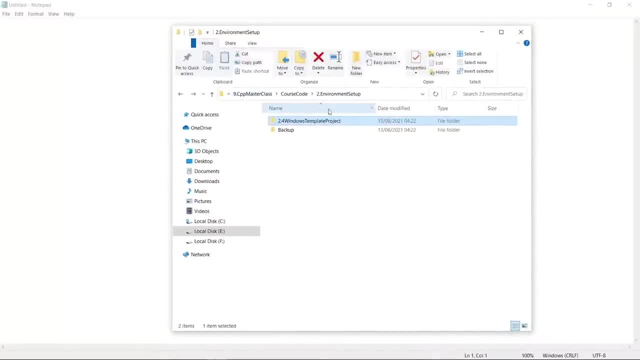 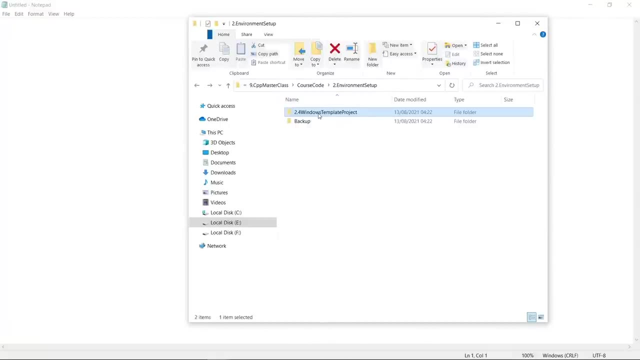 What I am going to do is really set up a template project we are going to be reusing throughout this course here. So I am going to go on a folder in my system and I am going to right click on the folder and say open with Visual Studio Code. 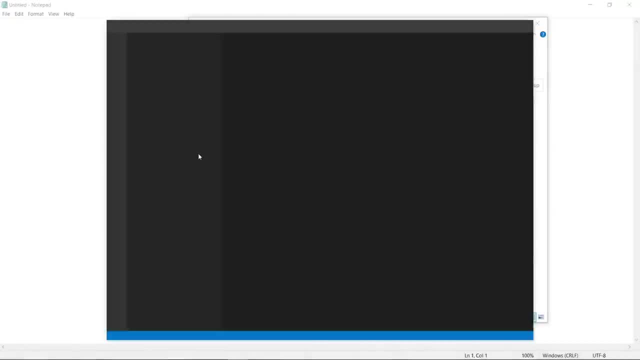 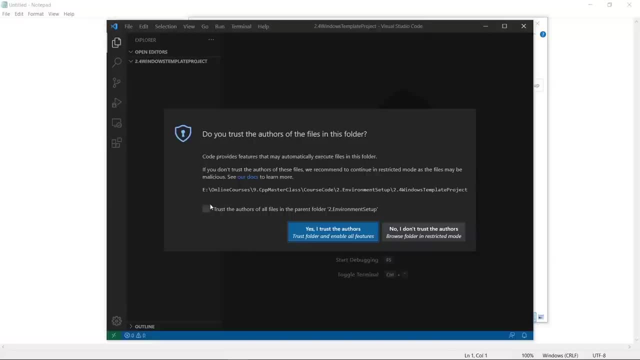 Let's do this. This is going to open this folder in Visual Studio Code and I am going to trust this folder here. Be careful what you trust, because some things are going to do some malicious things on your computer. Make sure you trust the folders that you open up. 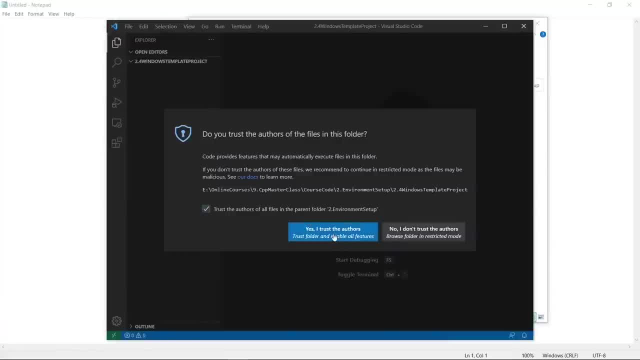 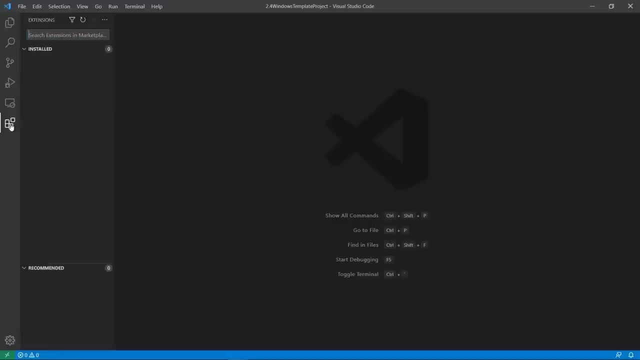 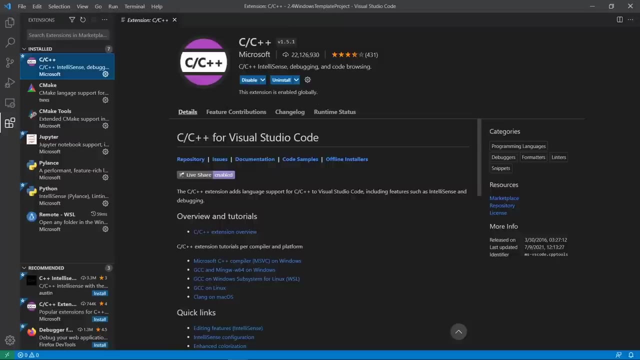 So I am going to trust myself, because I am the creator of this folder And this is going to open Visual Studio Code. Now, in our install video, we installed the C++ extension for Visual Studio Code. Again, if you don't have this installed, please make sure you go back and install and make sure this is saying that this is enabled. 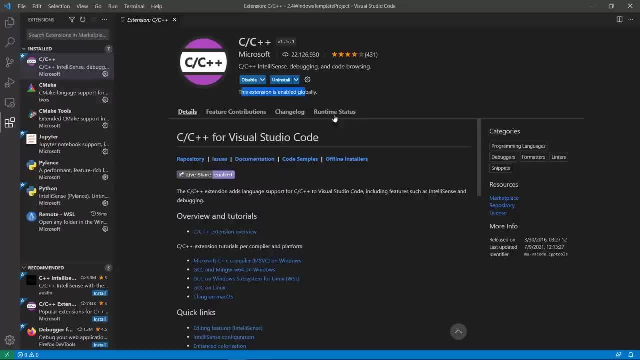 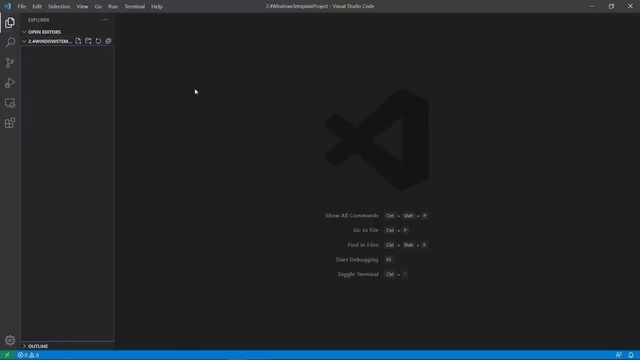 And now we want to use this to write C++ applications. Here we are going to write a simple TOY C++ application to just test that our compilers support C++ 20.. And then we are going to use this as a starting point or as a template project. 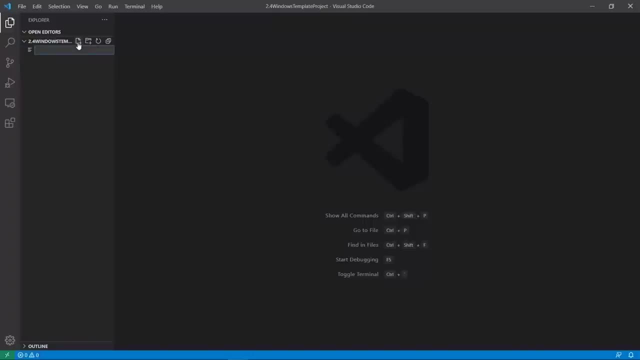 So I want you to click on this little plus icon here, And we are going to create a file called maincpp, And once you do that you will be able to type C++ code in this here. So we are just starting out here. 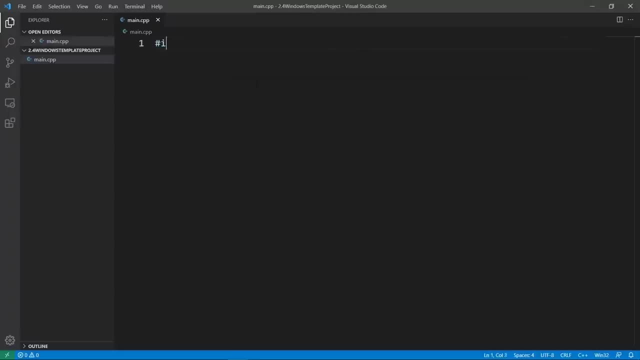 I would recommend to type this exactly as I do here: So we are going to say include And say opening angle bracket and say IO stream, And we are going to go down here and say end main And we are going to go inside these curly braces and say auto result. 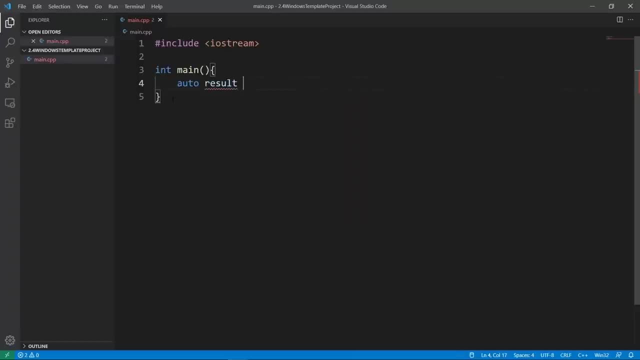 And you are going to exactly type what I type here. Don't worry, we are going to have a chance to learn about all these things here. So I am going to put a pair of parentheses and I am going to say 10.. And I am going to put a weird operator here. 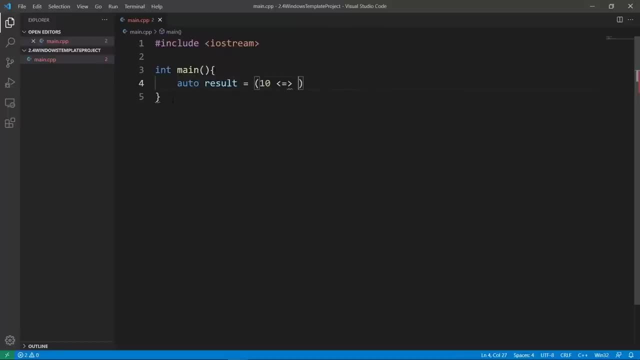 This is called the spaceship operator. It is just something we can use to test that our compiler supports C++20.. And we are going to put a 20 here And then we are going to try and see if this is greater than 0.. 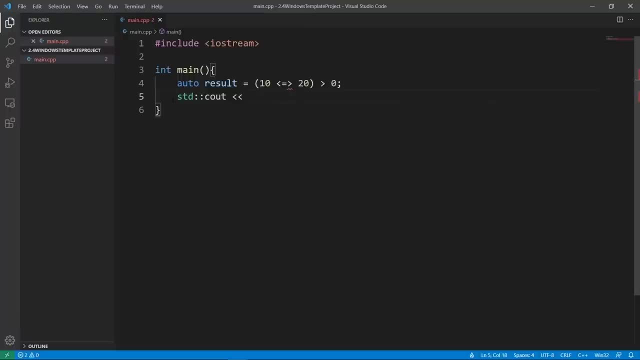 And we are going to print this out. We are going to say stdc out Again. don't worry if you don't know what this is. This is just a way for us to test and see if our compiler is going to be able to use C++20. 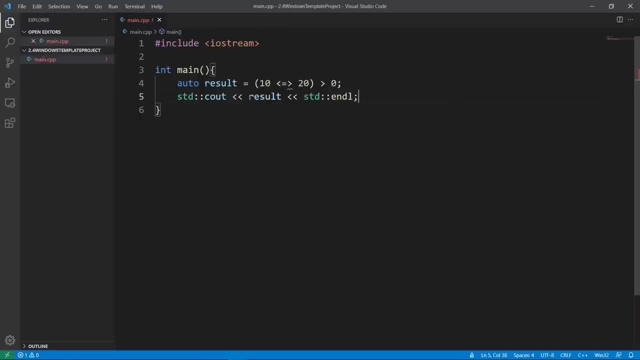 We are going to say result here And this is going to be our program. Now we want to make sure we compile this program. So to bring in your compilers in Visual Studio Code, all you have to do is come to the terminal menu here. 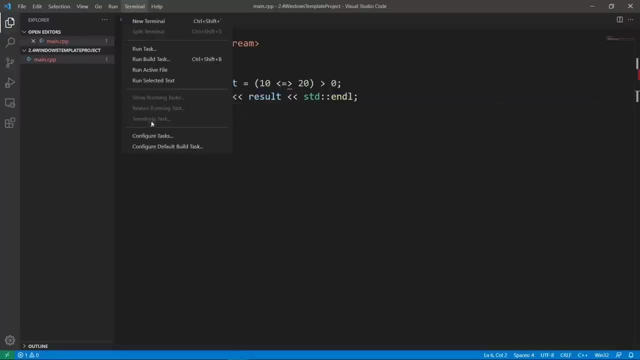 So please come here And we are going to have an option to configure tasks. I want you to click on this And once you do this, you are going to see that Visual Studio Code is going to find the compilers that we just installed. 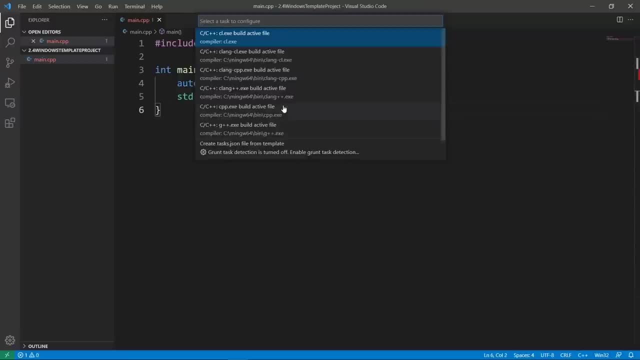 You see that it has found the GCC compiler we installed in MinGW. You see that it has found the Clang compiler. I know about the G++ compiler because you can see the path here. You can see cminjw-ben-g++exe. 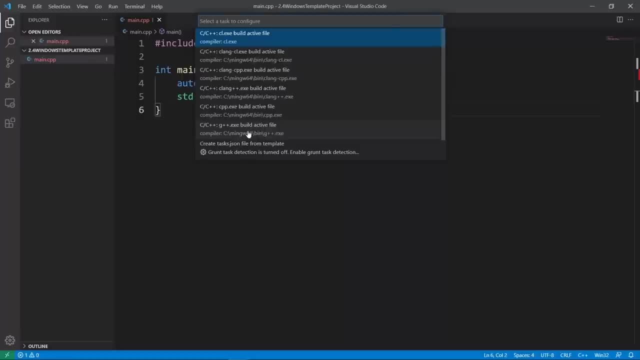 This is where we installed our G++ compiler, And I know about the Clang compiler because that's what's being found here. For example, on this entry here you see, it says cminjw-ben-clang++. So we want to configure these two compilers here. 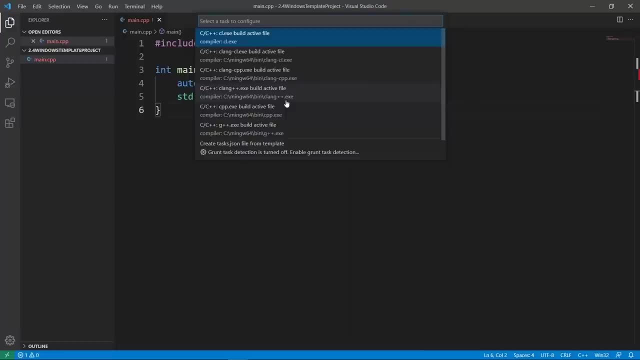 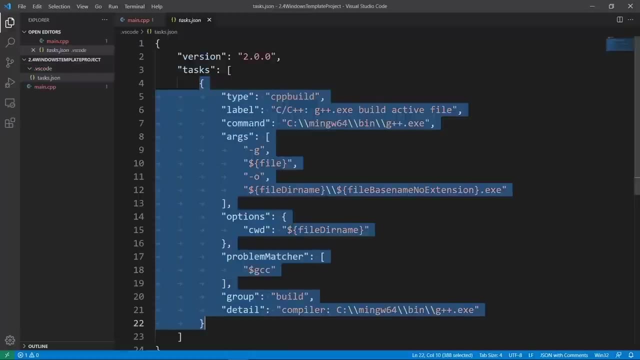 And let Visual Studio Code use this. Let Visual Studio Code use them to build our C++20 projects. Now what we're going to do is click on the G++ compiler first, And when we do that, this is going to create a tasksjson file in our project. 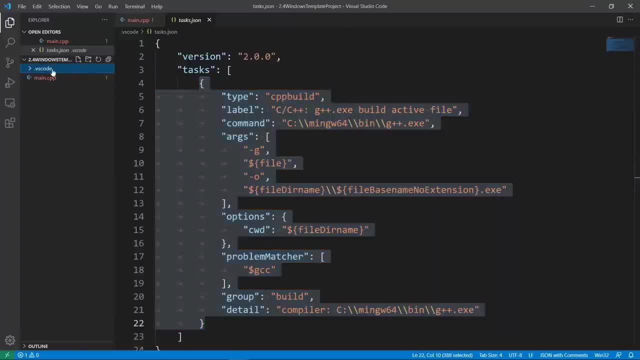 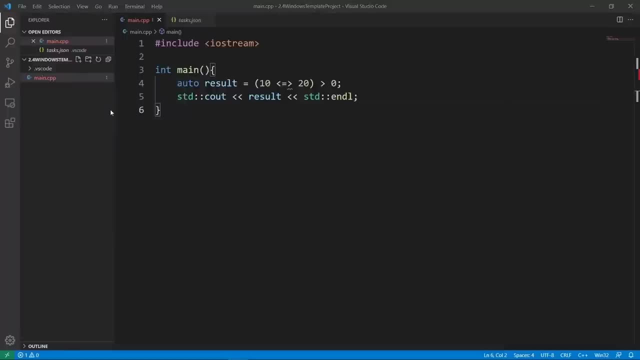 And you see that it has created a folder called vscode. If I click on my main CPP file here and do Reveal in Explorer, this is going to open up on my system And you see that this has created a vscode. 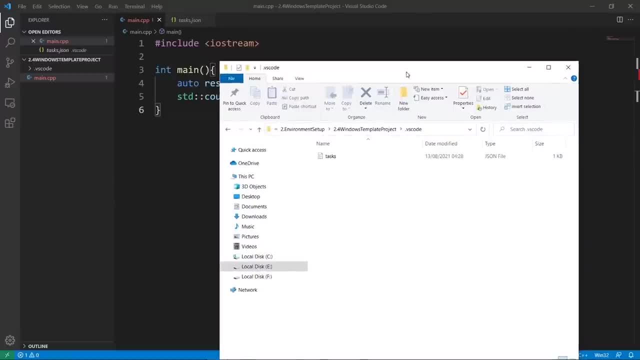 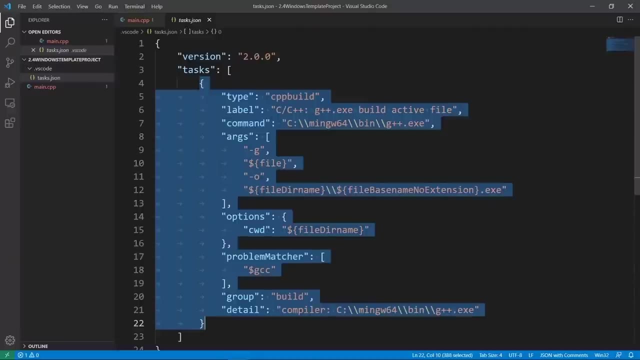 And if we go in, we're going to find this tasksjson file. This is going to be our configuration to configure which compilers that Visual Studio Code is using to compile our main cpp file here. So if we go in, it's going to really have everything ready for us. 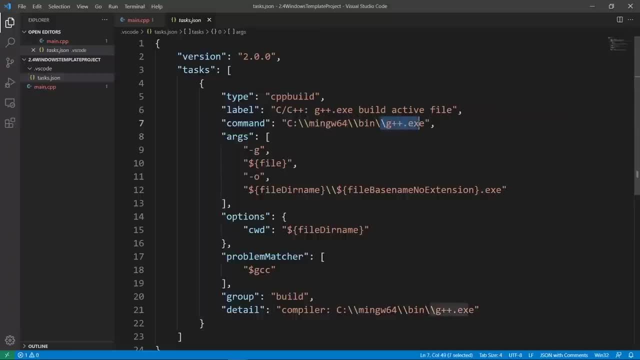 So you're going to see that it's going to be using our G++ compiler. This is the path to it, And in our args options here we have the options that we pass to the compiler to compile our program here. Now I want to change this to say which kind of compiler we are using. 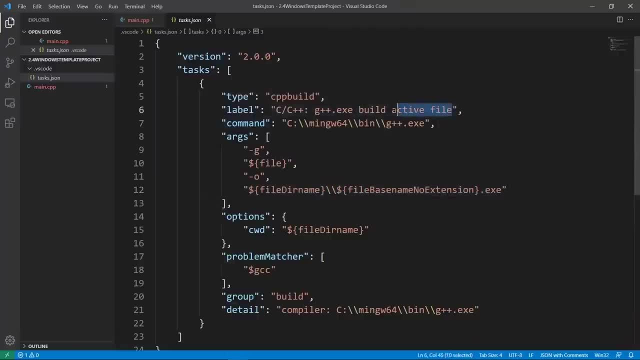 So we're going to change the level here to say world with G++ and save the version. I think that's going to be more descriptive here. So we're going to say world with G++ or GCC And we're going to say 11.2.0, because that's our version here. 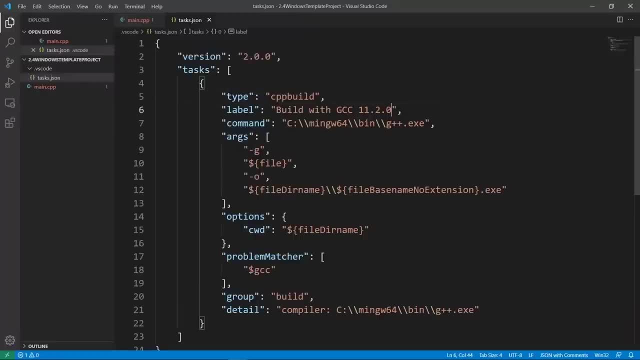 And the rest of this is going to be the same. The rest is really going to be enough. So let's try and see if we can compile our program here and see the thing here printing out. But the other thing we need to do because this program is using C++ 20,. 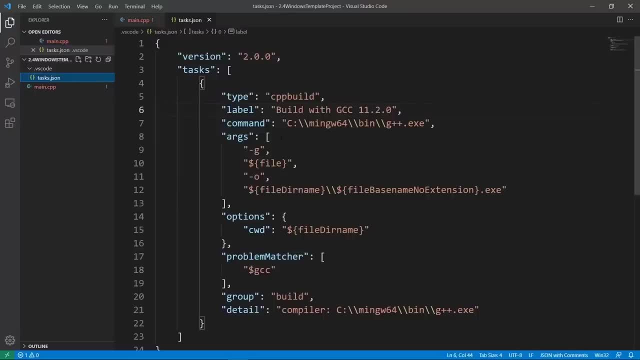 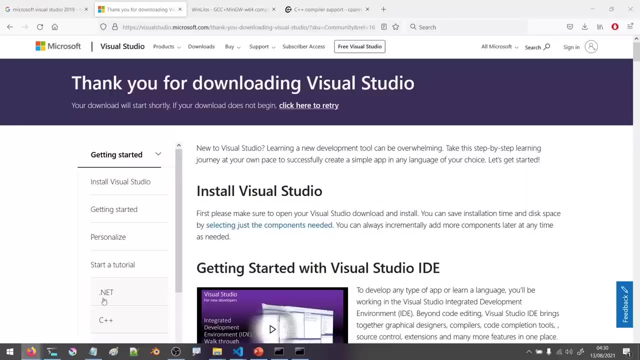 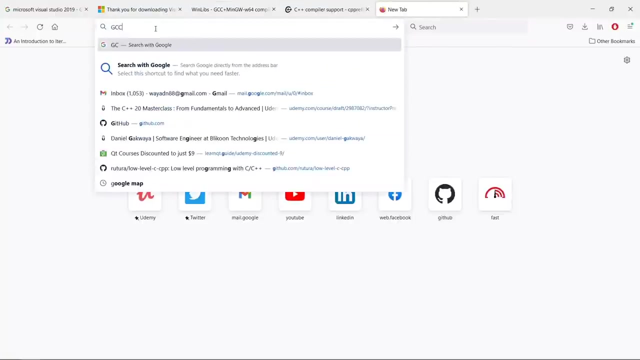 we need to configure our compiler to use C++ 20.. And one way to do that in GCC, and you can really search these things. For example, if we come to our search engine here and say configure GCC to use C++ 20, or even GCC and say C++ 20, you can search these things and find information. 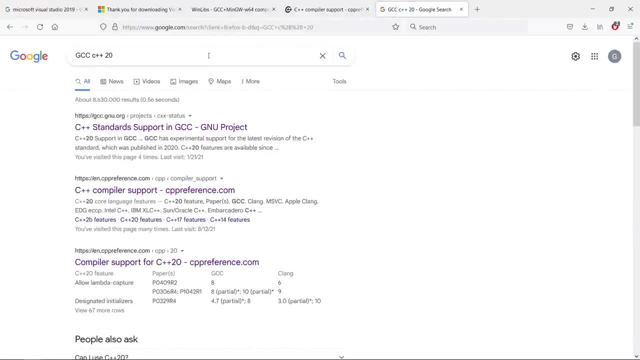 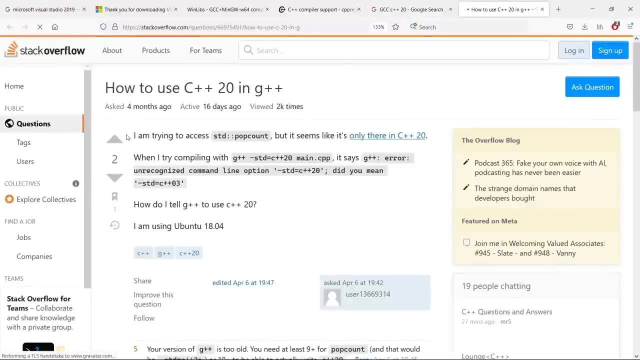 And it is a really good way to test your things here. So let's see if we can find a link to help out. We have a Stack Overflow link here so we can crack this open. And if we go and we're going to find a batch of things, for example, 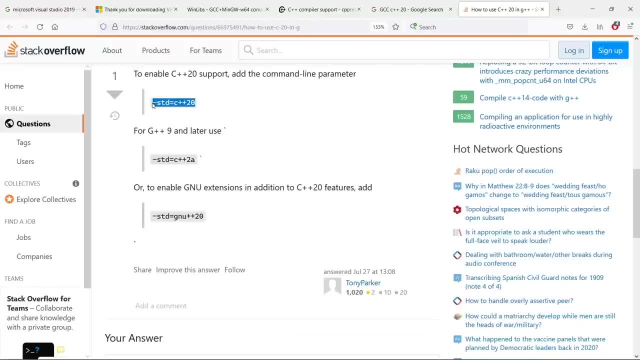 we can say STD C++ 20 here as an option to our compiler And this is going to bring C++ 20 support in our GCC compiler. So I am going to copy this and I am going to come back in my Visual Studio Code editor. 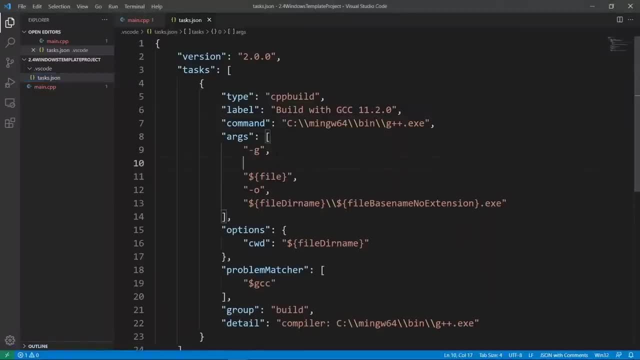 and I am going to pass a flag to world in C++ 20 mode And it is something I just got from Stack Overflow here And we are going to pass this to our compiler and put a comma to make this a valid configuration file. 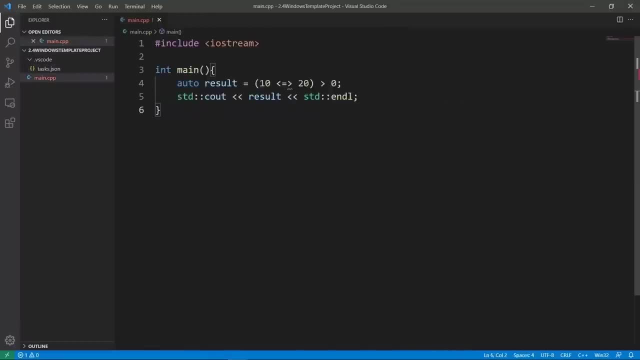 And I am going to close this Now: once we have this open and we want to build this, we need to bring a terminal window. So we're going to bring a terminal window so that we can see things happening, And we do that by coming to terminal and saying: new terminal. 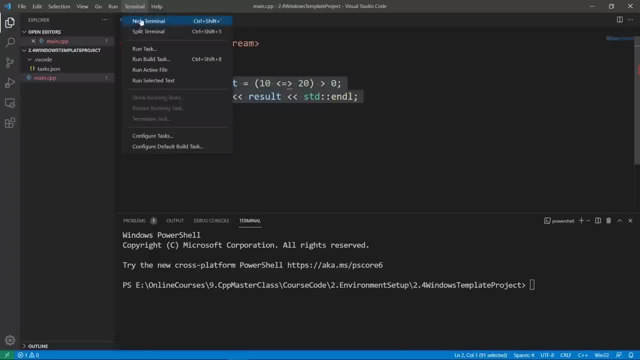 And we will come back to terminal again and say that we want to run a task. In this case, we're going to be running our build with GCC 1120.. Again, if you are using a newer version, that's what you should use. 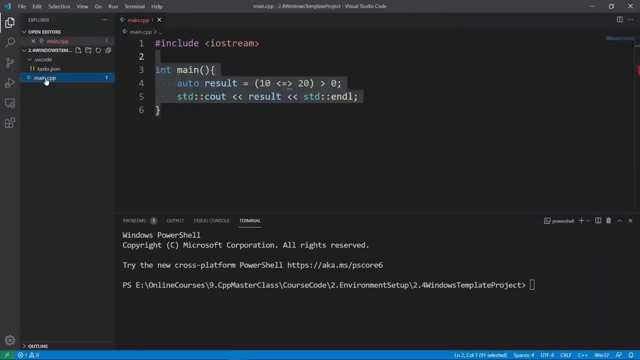 And if we click on this, then please make sure you have the main CPP file selected before you do this. So I have this selected and I'm going to go to run task And I am going to click on this little thing. You're going to see that this is going to kick off the process to build our program. 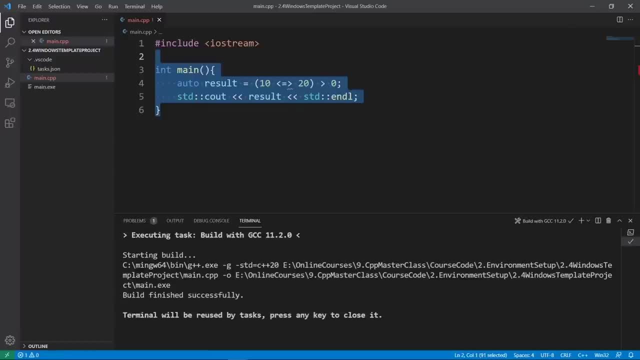 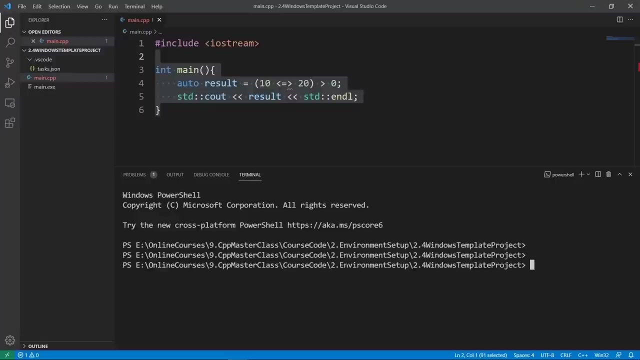 And we're going to wait for this to finish And you're going to see that it is using C++ 20 here We're going to see that the build finished successfully And we have a mainexe file created here. So if we go in our terminal in Visual Studio Code and click enter and type clear and hit enter, 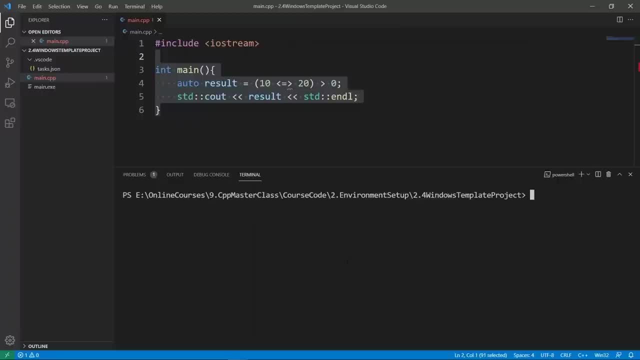 this is going to clear the screen. This is something you can do to clear things out. We can run this mainexe binary directly here. So we're going to run exe here And if you run it it's going to say zero. 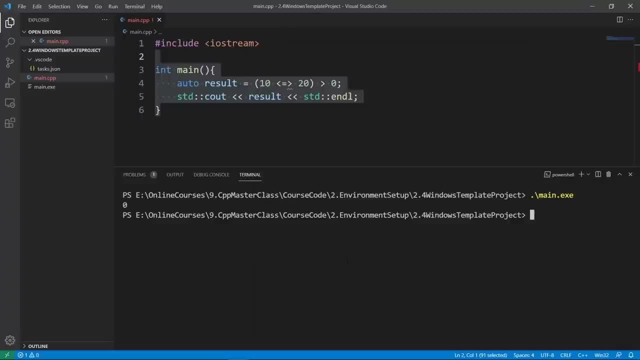 And this is an indication that we have our Visual Studio Code editor connected up to our GCC compiler And we can use that to compile C++ applications, And this is really the configuration we need. Now you may ask: how do I know this? 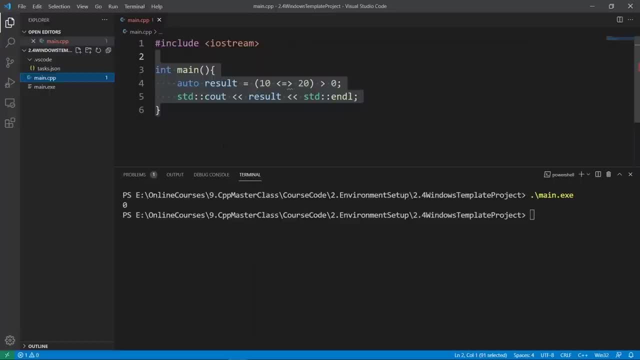 How did I know the steps to follow to get this to work? Well, if you come to extension tab here, and before we even do that, I want to bring to your attention that we have a bunch of tabs here in Visual Studio Code. 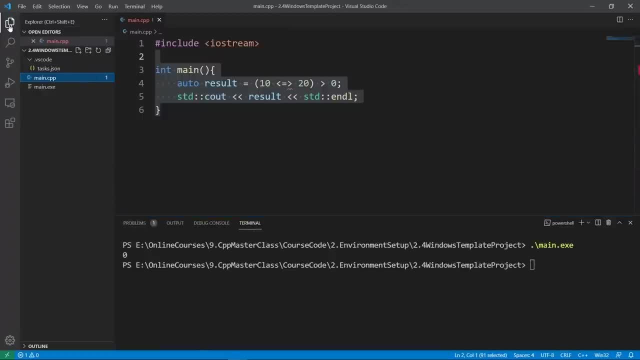 We have a tab that says file- I think The one here saying explorer. We have one we can use for version control. If you use something like Git or whatever, you can use this. But in this course we're mostly going to be using the explorer tab here. 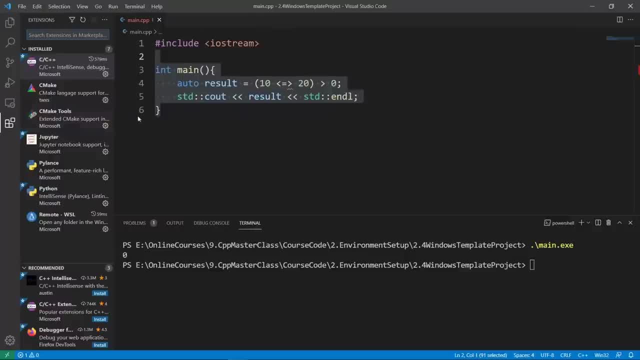 and the extensions tab to install this, And at a later time I will show you how to use the debug tab here or run and debug tab, But in most cases we're going to be using the explorer tab or the extensions tab here. 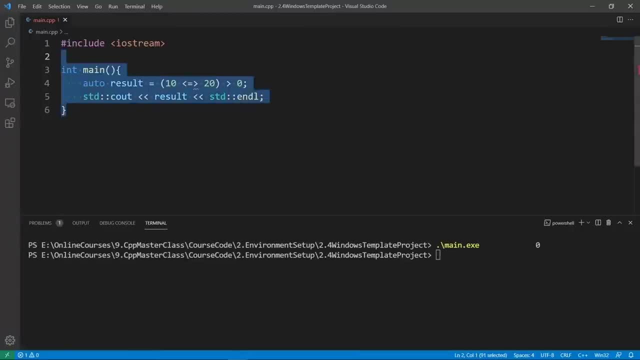 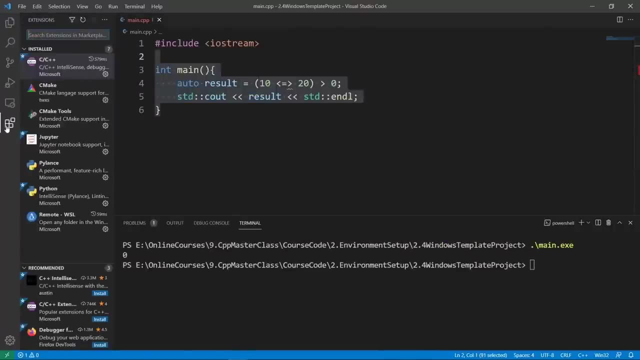 If you want, you can click on this to close this so that you have some more space. You can click again to bring this back. These are some things you can do in Visual Studio Code, But I am going to show you how to configure your compilers. where I got the information. 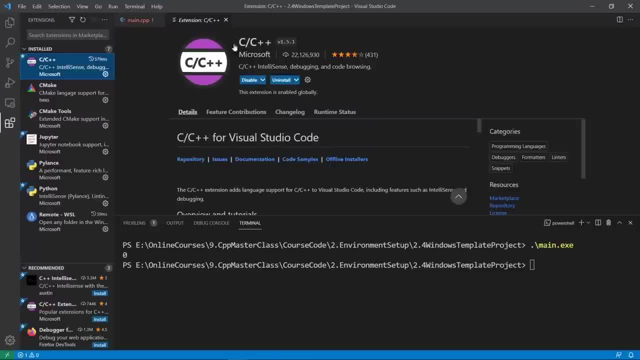 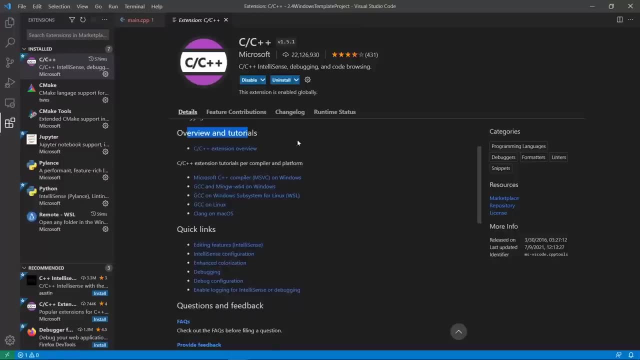 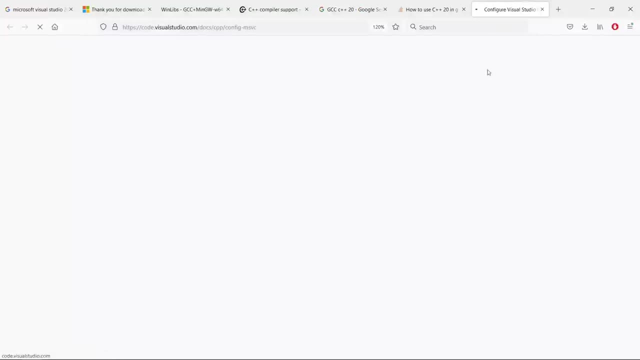 So click on extensions here And we're going to find our C and C++ extension. If we scroll down, we're going to find tutorials on how to set up this on different compilers. For example, you can crack this open to see how to set up Visual Studio Code to use your compiler from Microsoft. 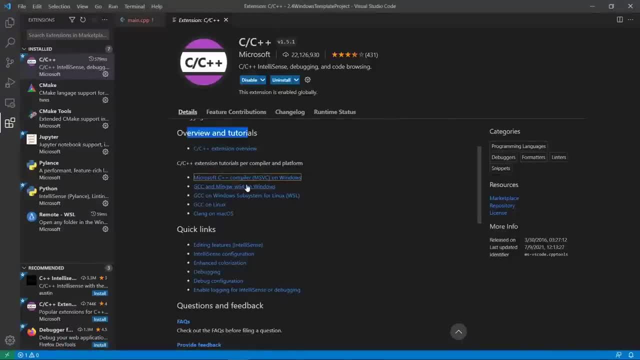 If we come back, we can see a link to see how to use this with main GW on Windows. Let's click on this And let's see what else we have We can come back to here And we can see how to use this with GCC on Linux or Clang on a Mac. 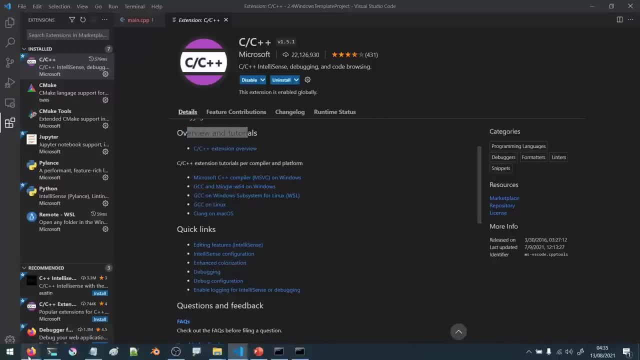 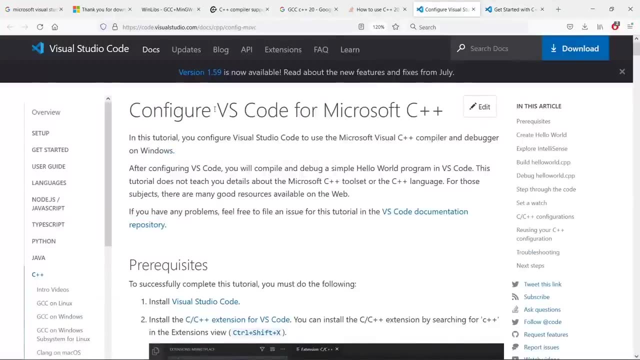 You can really choose whatever is relevant for your operating system, But in this case here we are just using the Windows operating system, So we're going to see how to use this with the main GW compiler that we just installed. Now we can use the main GW compiler. 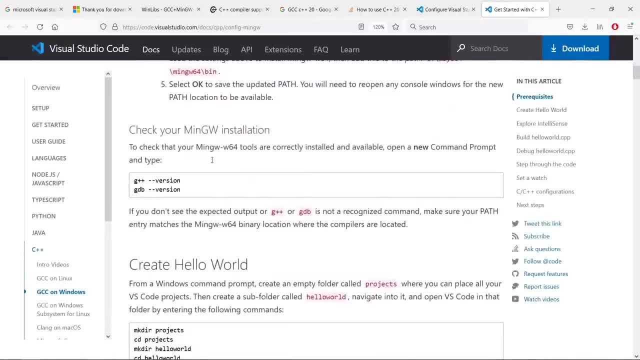 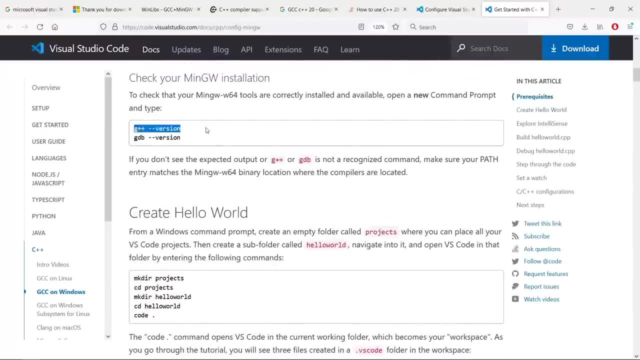 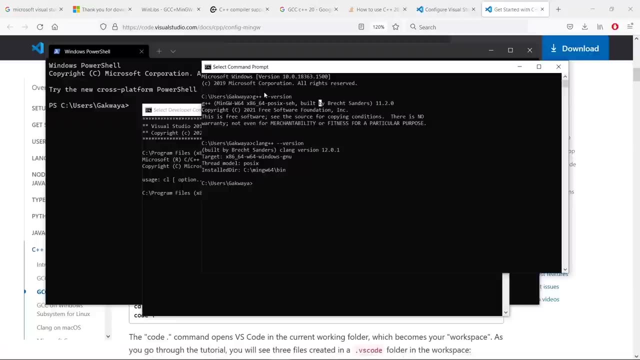 And I would recommend reading up on this entire thing to have an idea on what is happening. We already have our G++ compiler, So this command is going to work again. if we come back to terminal here And run G++ version, I think we can see that we run these commands here to see these things working. 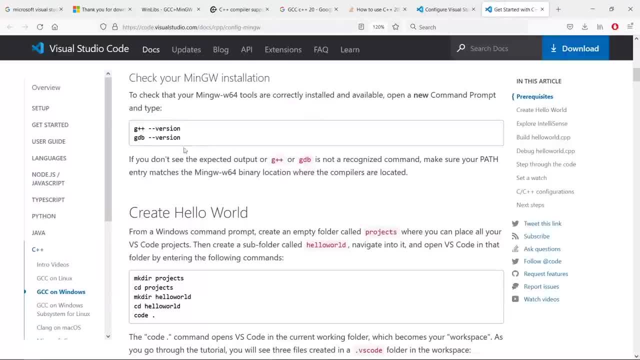 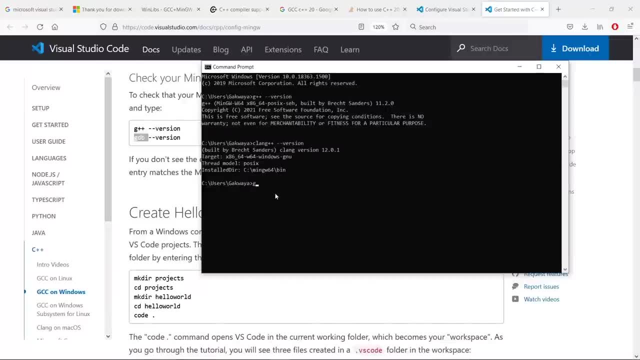 So we have this step here. And if you wonder what GDB is, it is just a debugger you can use to debug your programs. And again, if we come to our terminal here and say GDB, dash, dash version, we're going to have this available from our main GW installation. 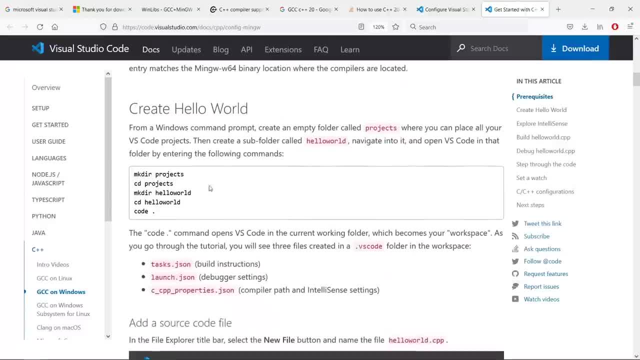 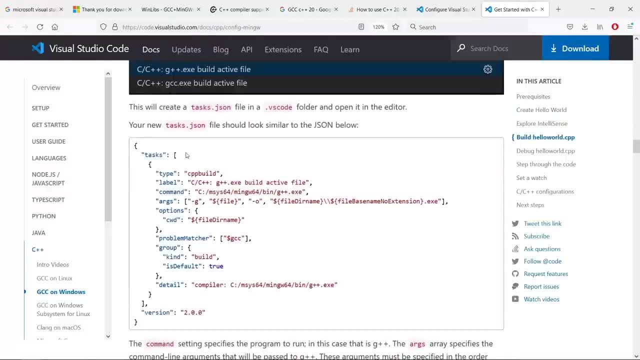 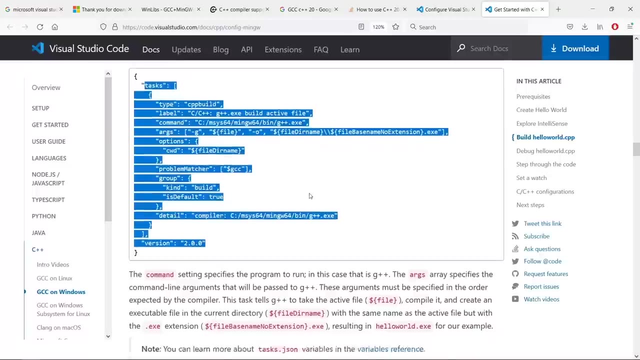 You can see that we have this here, So this is working just fine. You can really follow this and configure your Visual Studio Code installation, But I am just showing you how to do this pretty fast. You can see that this is what we set up in our configuration file, which is our tasksjson file. 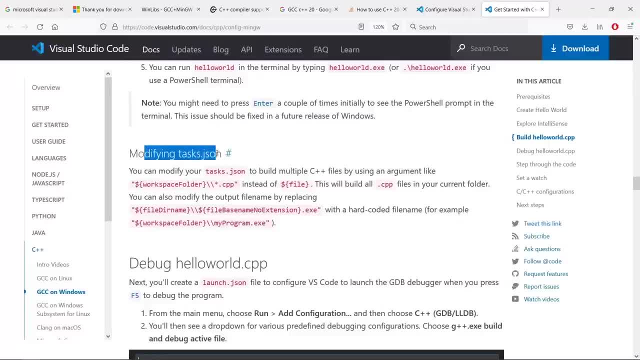 Now, one thing you can do is modify the tasksjson file to build every single file in your project, And this is something that is going to make things easier. What I am going to do is go back to our Visual Studio Code instance and find our project. 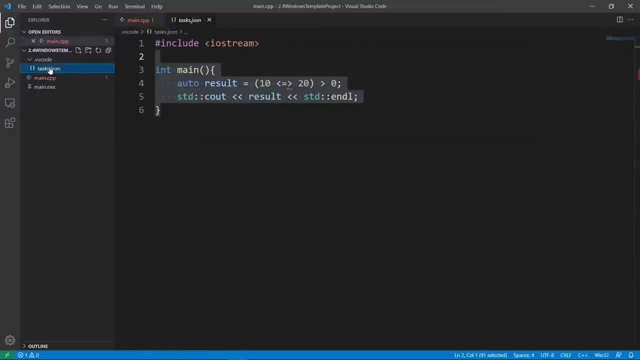 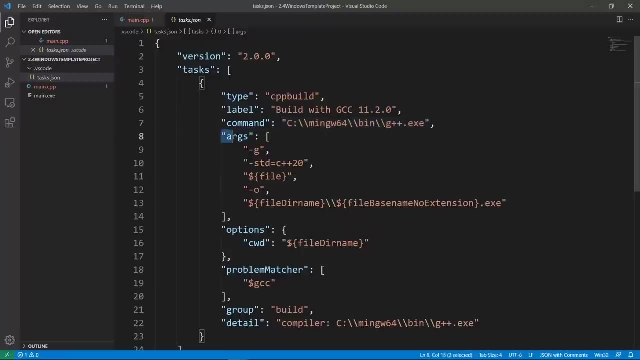 We're going to crack open our tasksjson file, which is living in our vscode folder, And I am going to take out the craziness I have in my arguments here. I am going to select everything I am going to delete that. 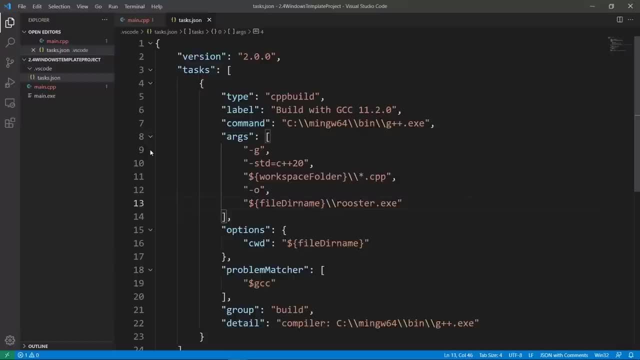 And I am going to put in a configuration that I am using for my projects here to make this super easy. What this is doing. it is telling the compiler to build in C++20 mode. It is going to tell the compiler to build every single CPP file in our project. 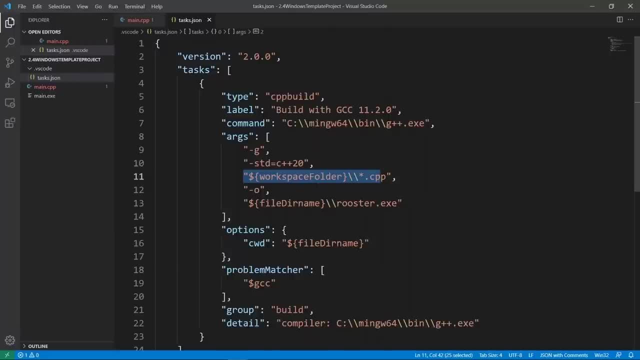 So if we have multiple files, they are going to be built together And we're going to specify the name for our output file. For example, if we don't want our binary executable to be named mainexe, we can give it a name. 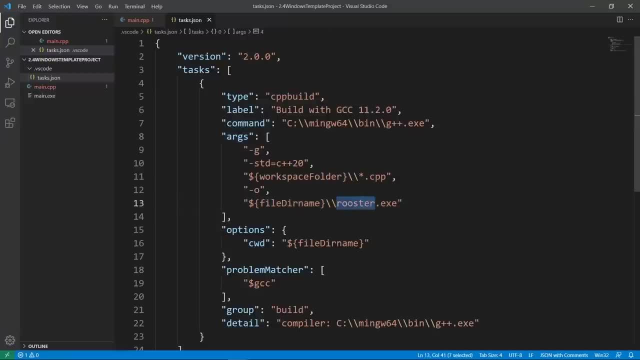 And I am going to be naming mine roosterexe in the course here. I would recommend doing the same so that we can really have the same habits as we go through the course here. But of course you are free to use whatever you want in your C++ programs here. 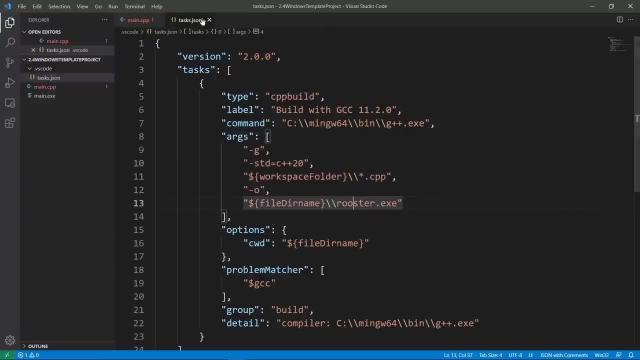 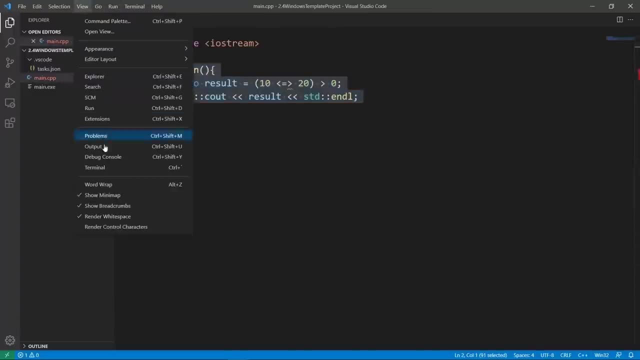 So once you have this, you can click save here And this is going to save our JSON file here. I can close this And I am going to bring my terminal by going to view and terminal here. This is going to bring back my terminal that I had before. 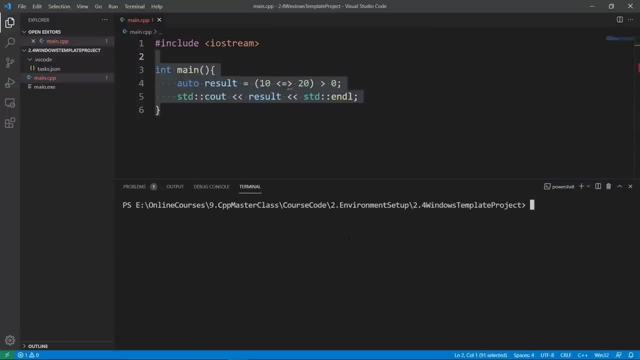 And I am going to run the clear command and hit enter And I am going to do DIR to show the contents of my folder on Windows. here I want to remove the mainexe file from the terminal, So what I am going to do is say rm. 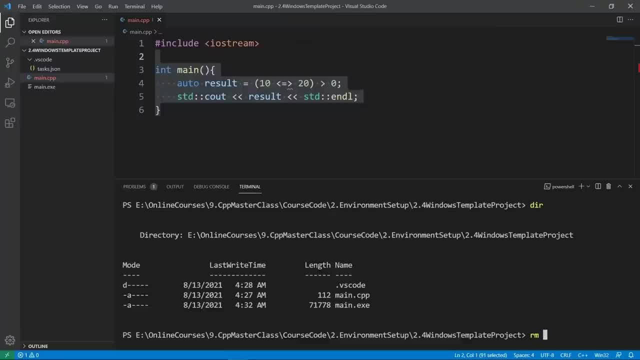 And I am going to say the name of the file I want to remove. I am going to say mainexe. And if I hit enter, notice what is going to happen: The file is going to go away. I don't see it anymore here. 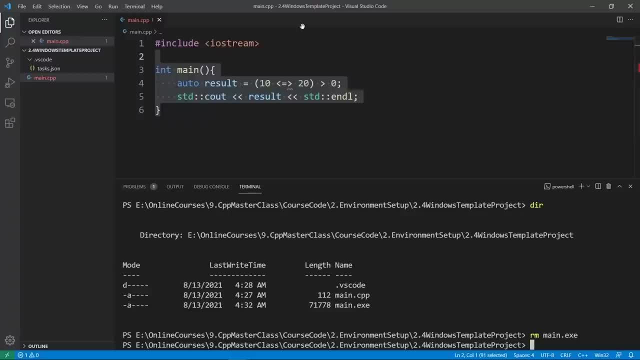 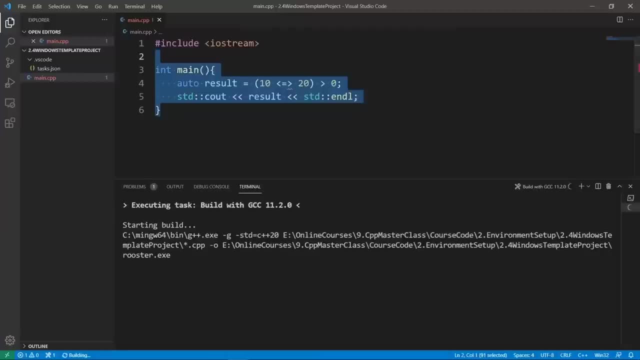 I want to build again using my new configurations in my tasksjson file. I am going to run the task to build with our GCC compiler. This is going to build again And you see that it is using the configurations that I passed. You see that it is building every single CPP file in the directory here. 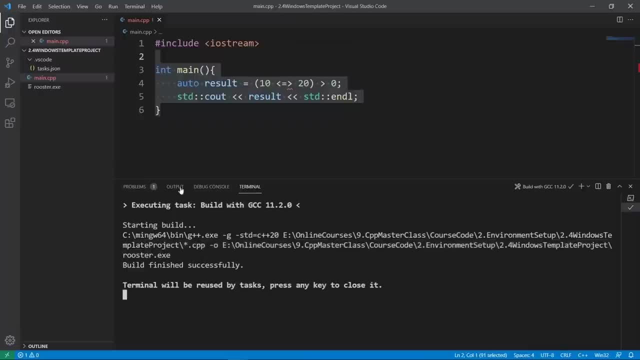 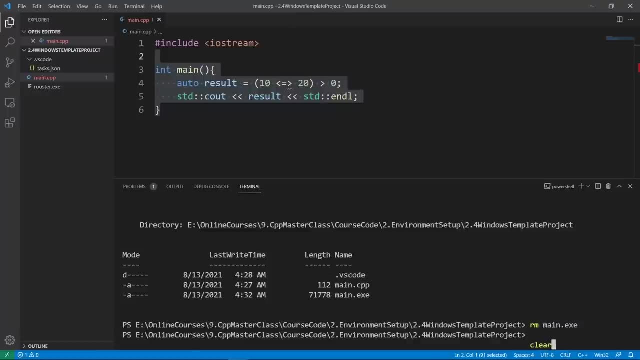 And it is going to generate a program called roosterexe. And if we look here we are going to find it. We can hit enter in the terminal And we can type clear to clear things out, And if we do DIR again, we are going to see that we have roosterexe. 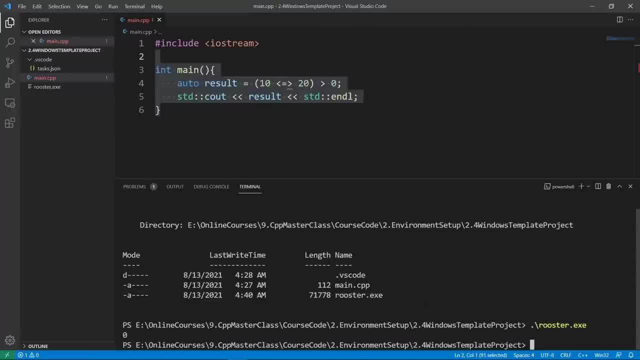 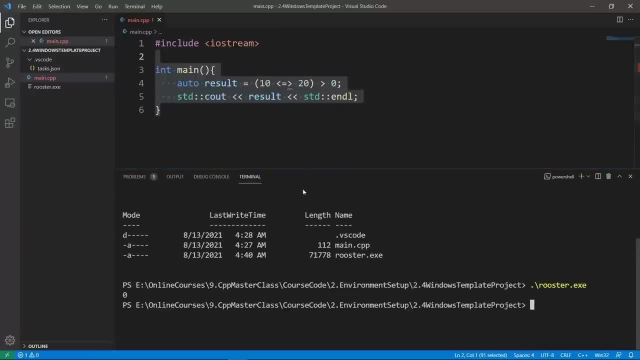 And we can run it by doing roosterexe here, And this is going to do what we want. This is really all you need to do to connect Visual Studio Code to your GCC compiler. Now we are going to connect Visual Studio Code to our Clang compiler that we have installed. 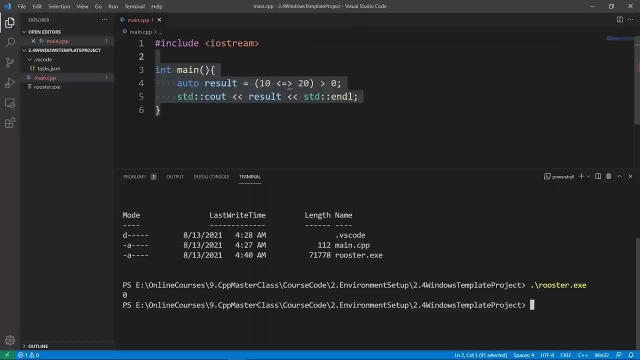 We really want to be able to use it with our project here And we are going to go through the same steps again. So we are going to go to terminal and say, configure tasks, And we are going to choose something that says the Clang compiler. 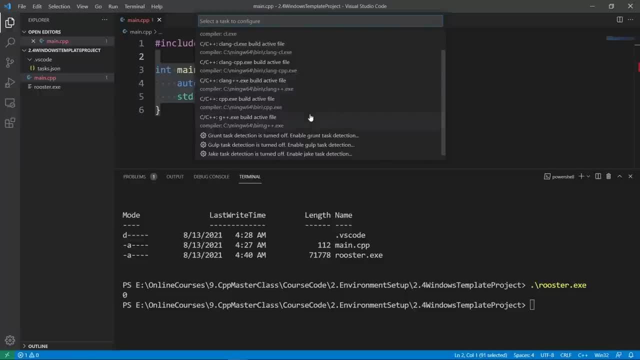 And we are going to find Clang++, So let's hunt for that. I have something that says that here We have clang++exe. I am going to click on that, And if I do this, this is going to add an entry in my tasksjson file. 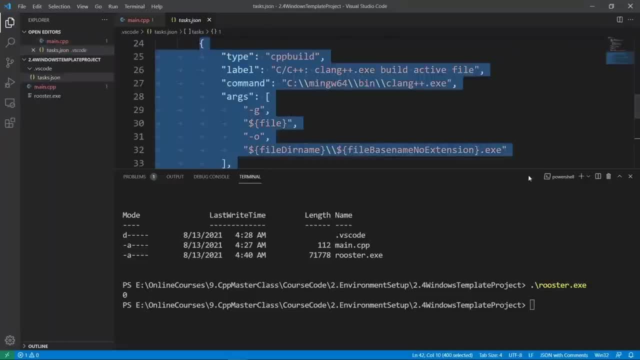 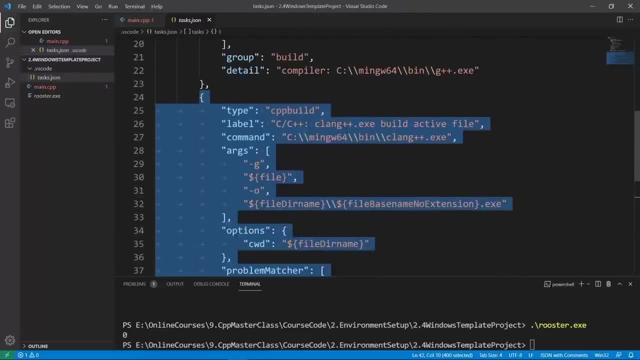 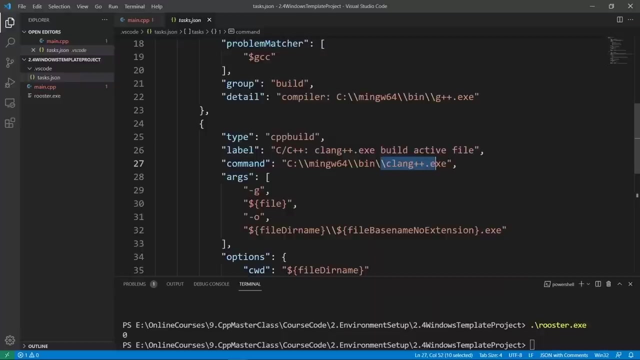 So watch out for this. I am going to click on this And let's crack this tasksjson file open And you are going to see that this is going to also set up another configuration to world using my Clang++ compiler, And again I can edit this out a little bit to say what we want. 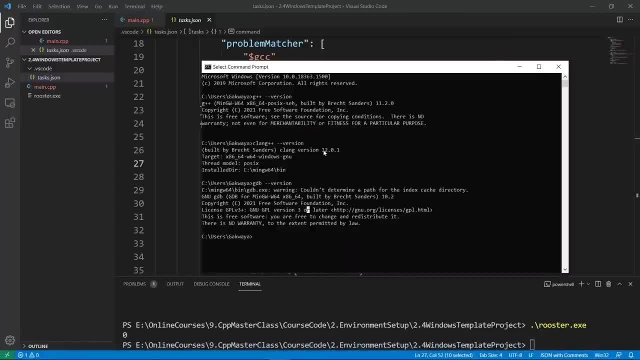 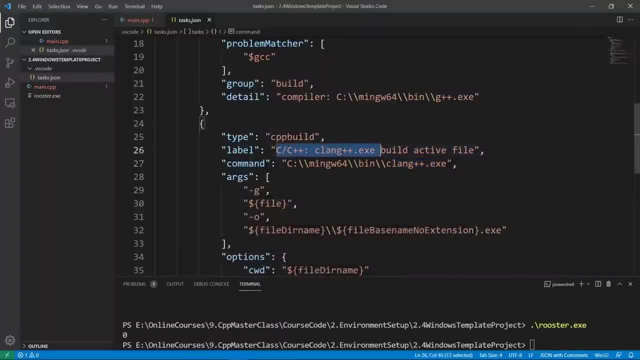 Let's look at the version of Clang we have installed to say that out. This is going to be 1201.. So we are going to say world with Clang++- 1201.. Let's say that here in our label: 12.0.1.. 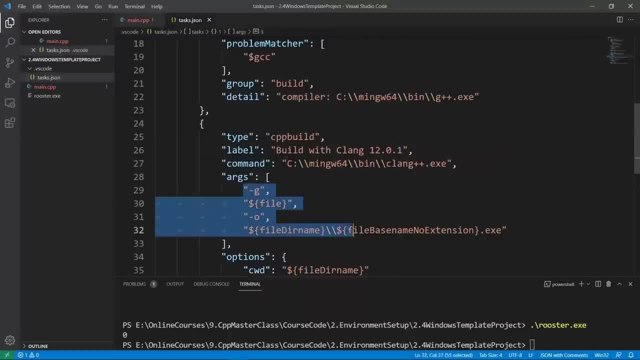 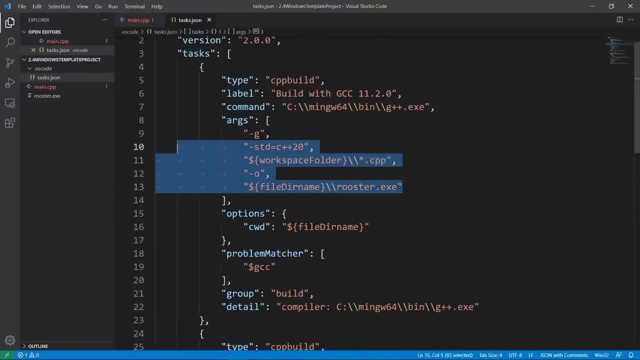 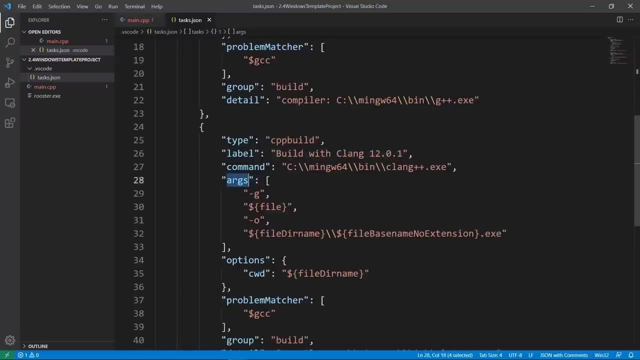 We can say that right here And you see that it is really doing the same thing we did with our GCC compiler. So what I can really do is I can steal everything I did in my GCC compiler. I can copy this And I am going to take out the arguments I have in my args here: 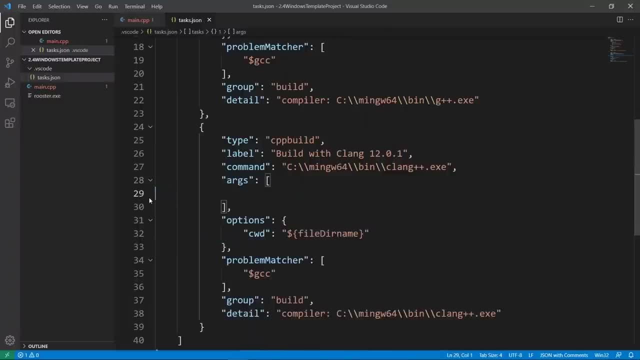 And I use what I have in my GCC compiler. You can see that you can use the Clang compiler and the GCC compiler in the same way, And this is something really cool. So now we have the option to use two compilers, And this is really cool. 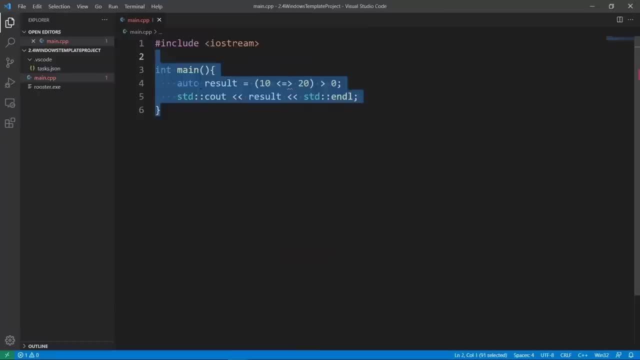 So we are going to close the JSON file and it is going to be saved automatically, And we are going to bring up our terminal window again- And let's bring this up a little bit- And we are going to do DIR on Windows And we are going to remove the binary again. 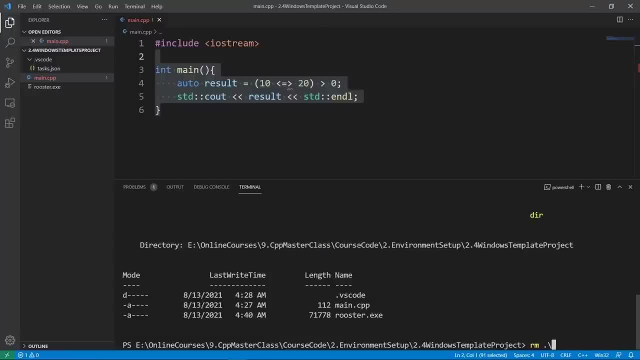 We are going to remove rasterexe. And again what you can do: you can start typing the name of the file you want to remove And hit tab. if you do that, The terminal is going to auto complete this for you, And this is really cool. 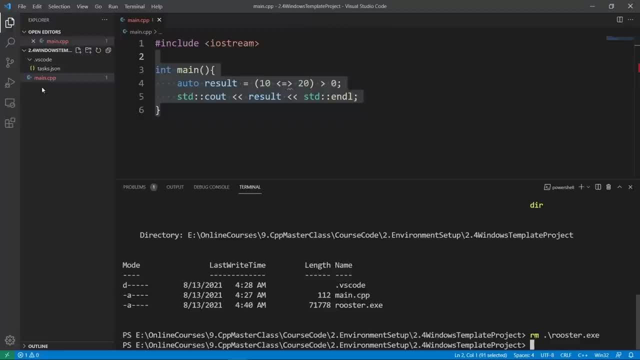 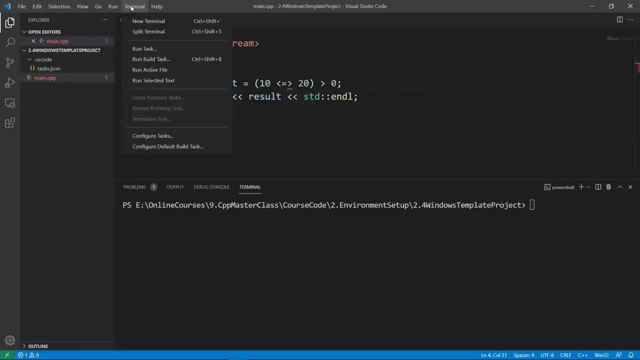 So if I do this, the file is going to go away. You see that it is gone right here And I can clear And what I am going to do is build with the Clang compiler. I can do that by coming to terminal. 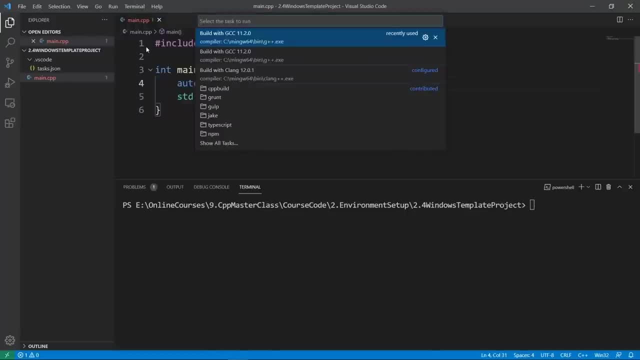 I am going to say that I want to run a task And I am going to be given an option. I can either build with GCC, So if I choose GCC here, it is going to be used, But I can also use Clang. 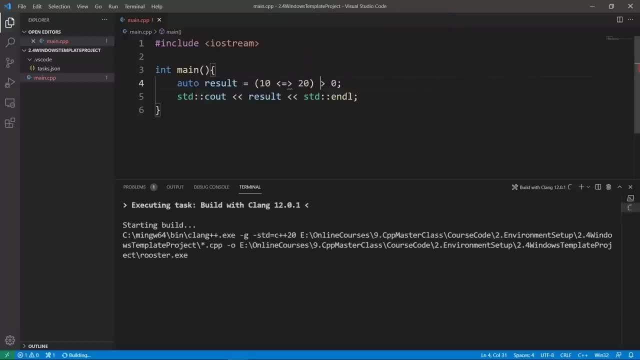 Let's use Clang here. So I am going to click on this And you are going to see that Visual Studio Code is going to kick off the build process. This is going to build my binary. It is executable And notice that it is using C++20 again. 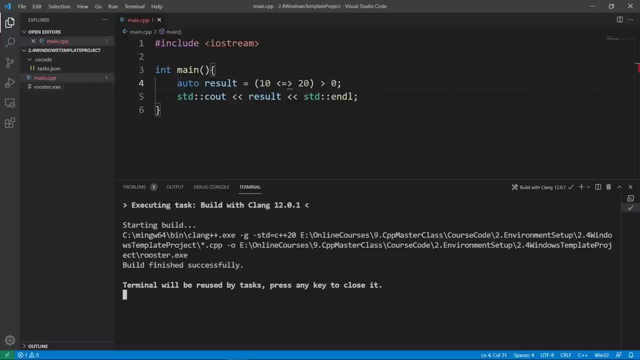 The build is going to finish successfully And I will have a binary here And this is going to be all I need to do. So if I hit enter and run my binary by tapping the name And hitting tab, this is going to auto complete. 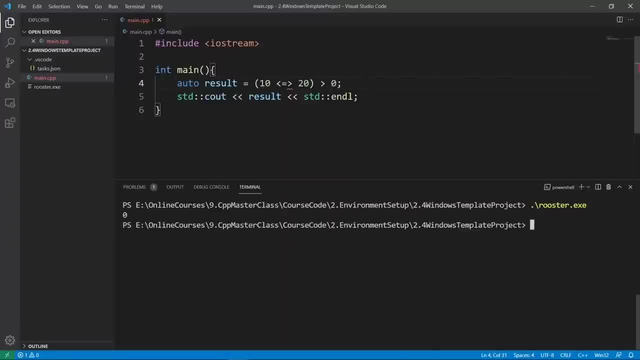 If I run it, it is going to say 0. And this is what we expect here. If you have some kind of error, please try and fix it. If you have a problem, you can ask me And I will do the best I can to help you out. 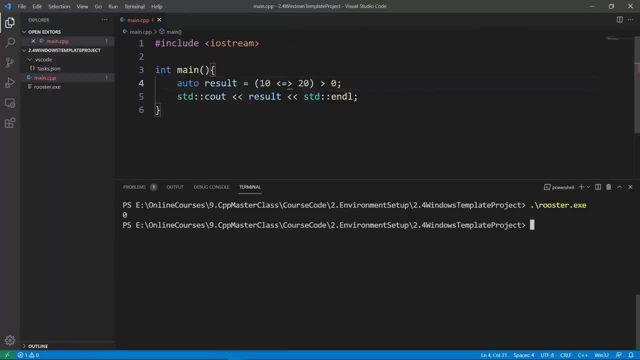 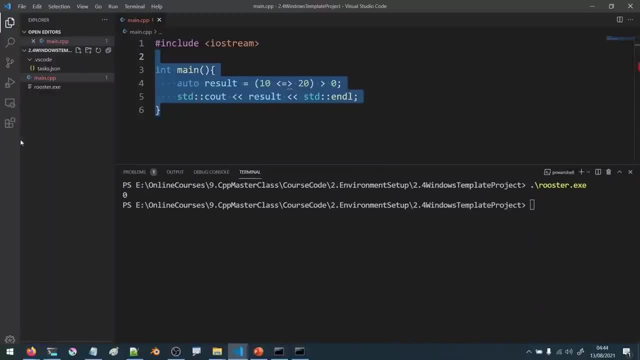 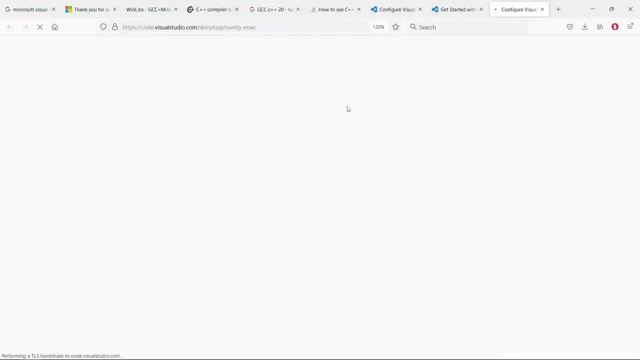 Okay, now we have our two compilers working, We need to configure the compiler from Microsoft. Now, the compiler from Microsoft is a little bit weird Again. you can read up on this by coming to your extension documentation And going to using the compiler from Microsoft with Visual Studio Code on Windows. 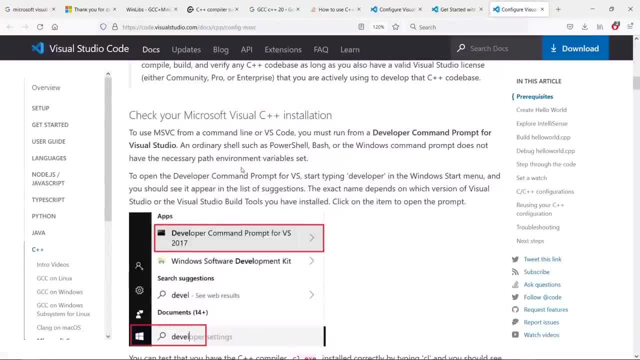 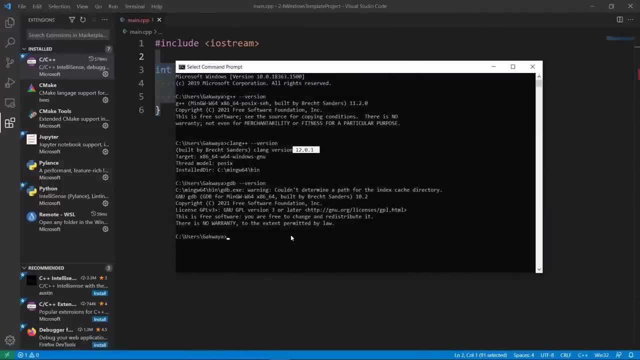 You can read up on all this if you want, But I am just going to show you a quick way to get this running. So the compiler from Microsoft is special in that you have to specify the path to it. For example, if we open a regular terminal window and say clexe to call the compiler. 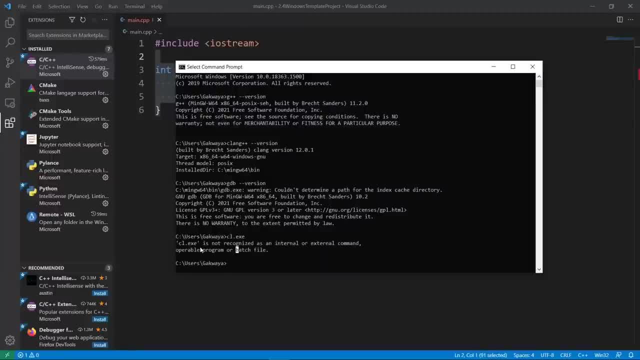 We are going to see that the terminal is going to say that the clexe compiler is not recognized And the reason is we don't have the proper environment variable settings for the operating system to find this compiler. when we call it right here We are able to use G++ and Clang because we put the environment variables in place. 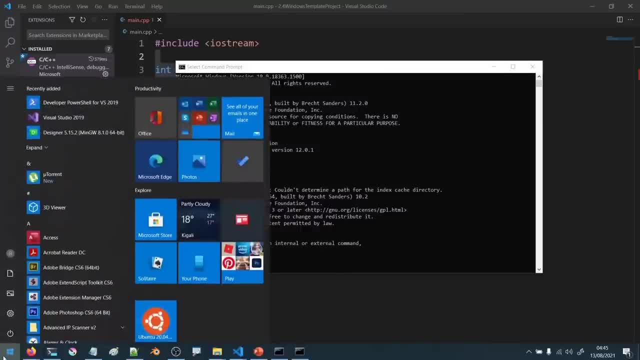 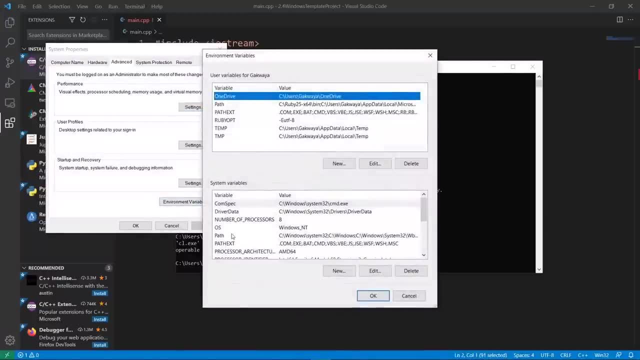 If you remember, when we installed them, we did something like this: We came to the start menu and did env, We came to environment variables here And we put the path to our compilers in our environment variables here. You can see them right here. 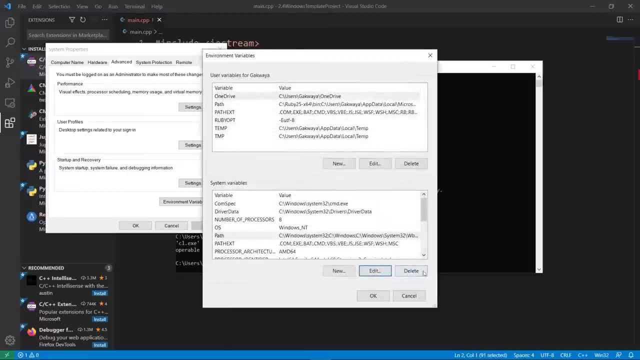 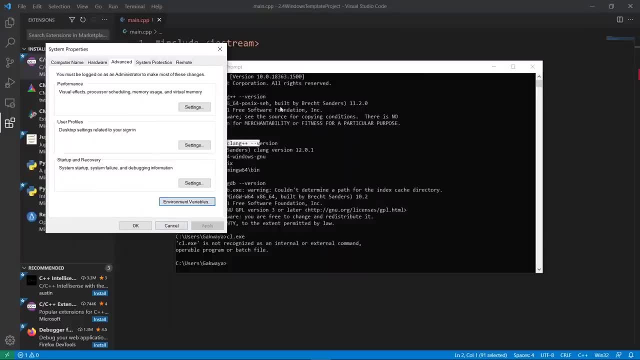 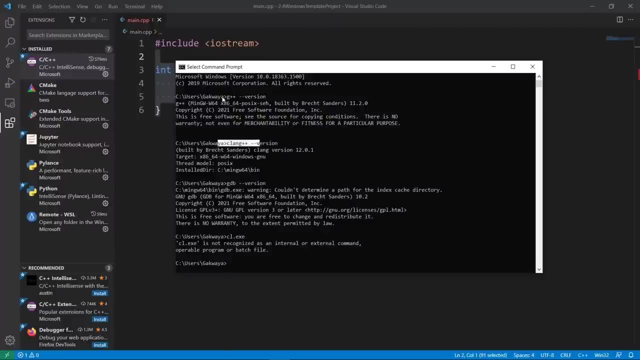 So we don't have the same thing for the compiler from Microsoft, And that's for a reason: Because we have multiple compilers installed from Microsoft. Then, if you have multiple compilers, it would be really cumbersome to choose which compiler you want. The guys at Microsoft opted for the option for you, the developer, to specify which compiler you want to run by coming to the start menu here and typing developer. 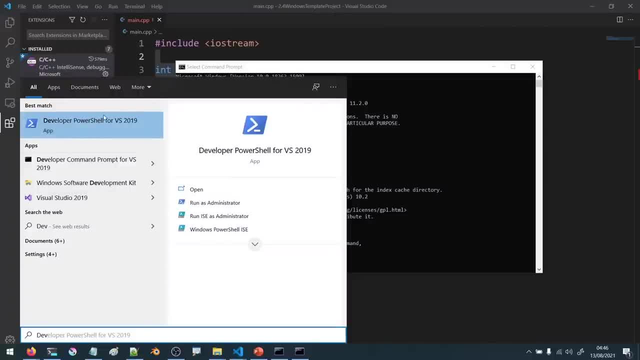 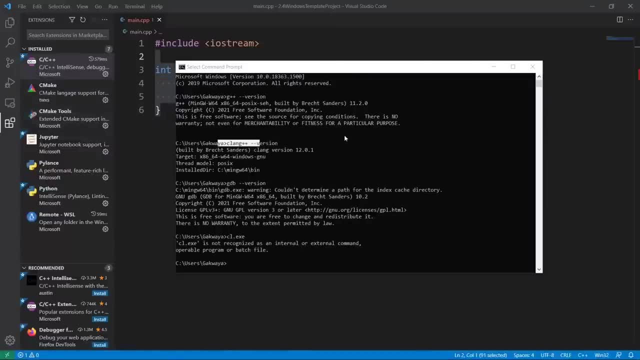 And choose which PowerShell for the compiler you want to use. For example, if we want to use the Visual Studio 2019 compiler, we can click on this And then we will have a terminal that can run the C++ compiler from Microsoft. 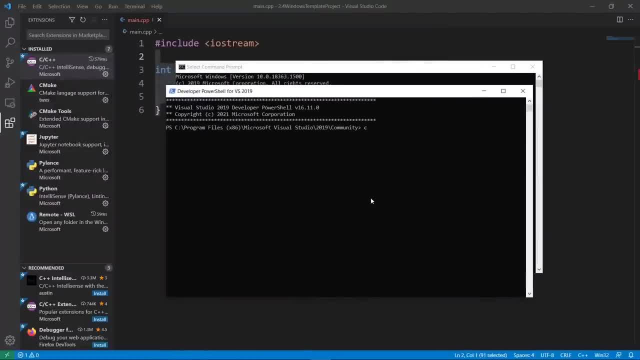 For example, if we wait for this to be ready and say We're going to see that we're going to have a message saying that this is our compiler, We can use it however we want. So what we're going to do is set up a terminal like this and use this terminal to start Visual Studio code. 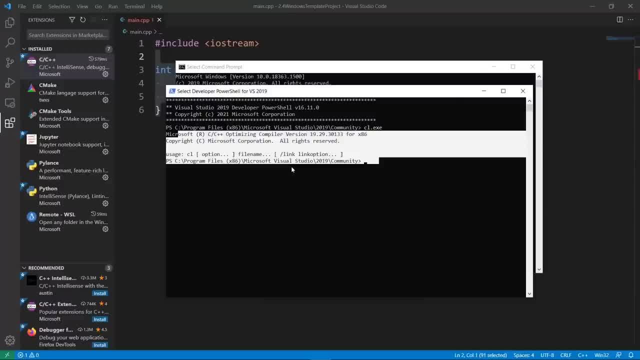 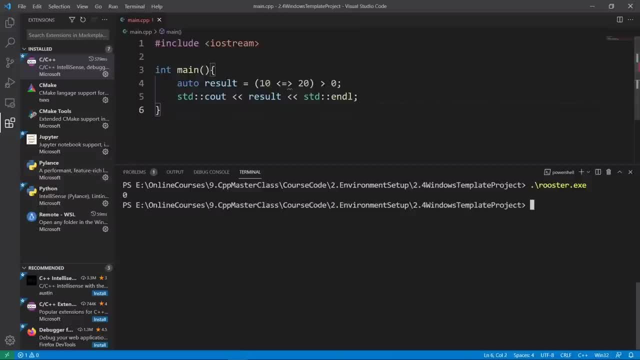 And the Visual Studio code is going to start in a mode where it can find the compiler from Microsoft. I know this is confusing, but please bear with me. This is what we need to do to get this to work. If we start Visual Studio code in a mode where it knows about the environment, 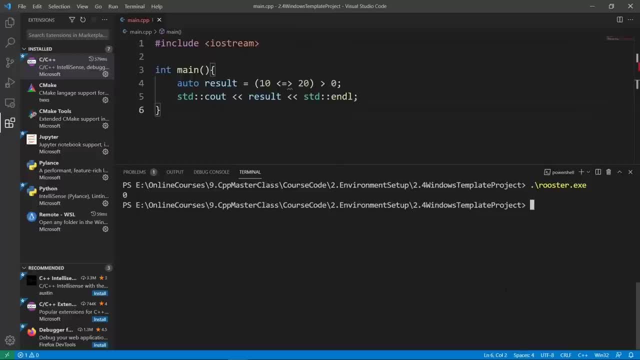 the environment variables for the compiler from Microsoft, we will have the ability to say clexe and we will be able to use that right here. But you see that it is not recognized now. But we can use the G++ compiler if we do this version. 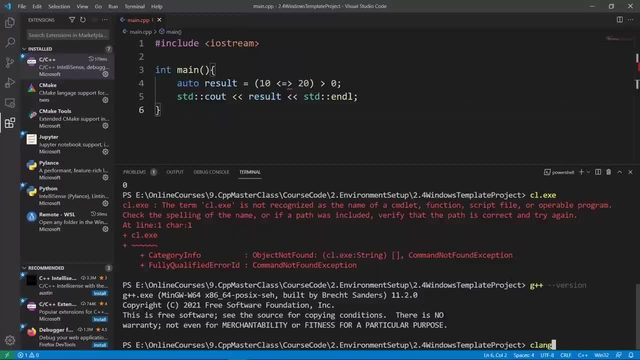 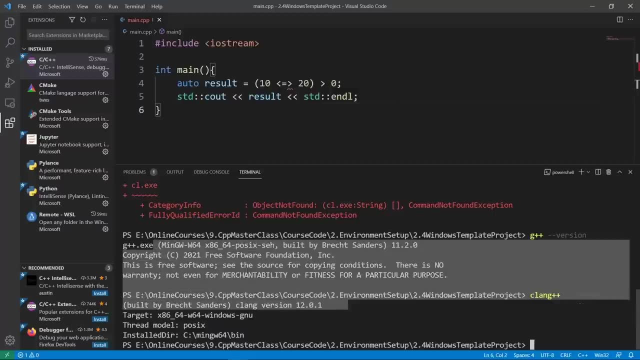 We're going to see that it's available. We can use it. We can use Clang++ And if we do version as well, we're going to see that we can use this little guy here. We also want the ability to use the compiler from Microsoft. 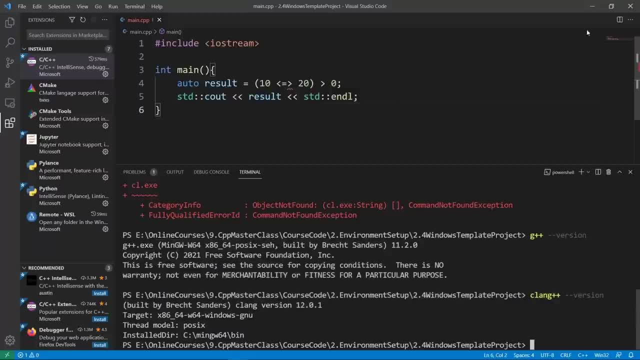 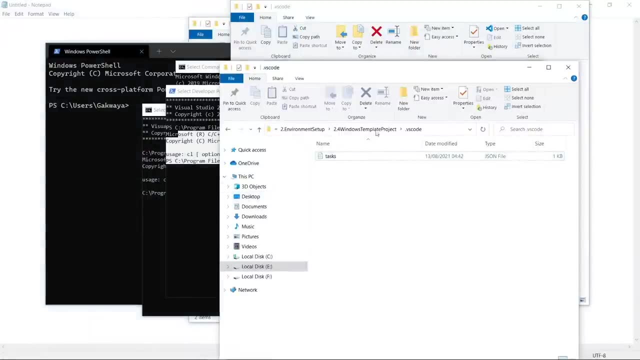 But to have access to that we will have to close the Visual Studio code instance we have here And we're going to come back to our project. Let's see if I can find it here. So we're going to go to the location where we have our project. 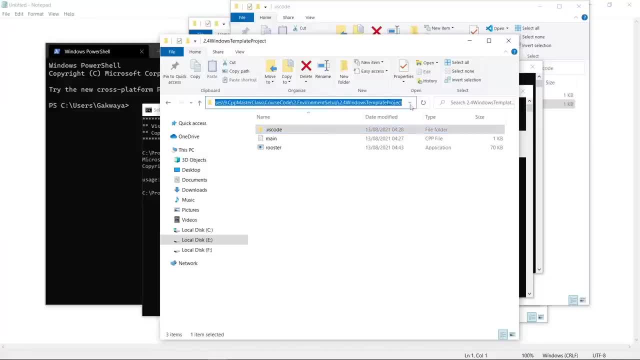 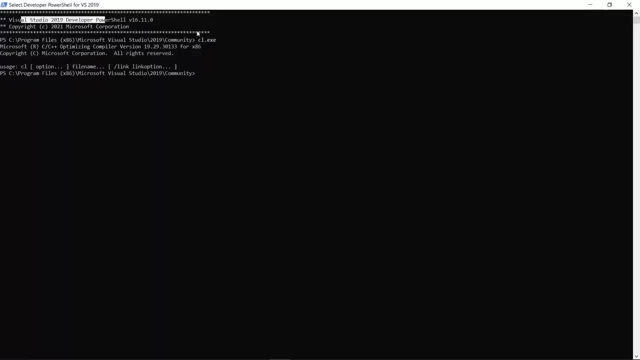 And we're going to change to the location of the project here So I can grab the location from my Visual Studio code project that I just set up. I am going to come back to my PowerShell window that knows about the path to the C++ compiler from Microsoft. 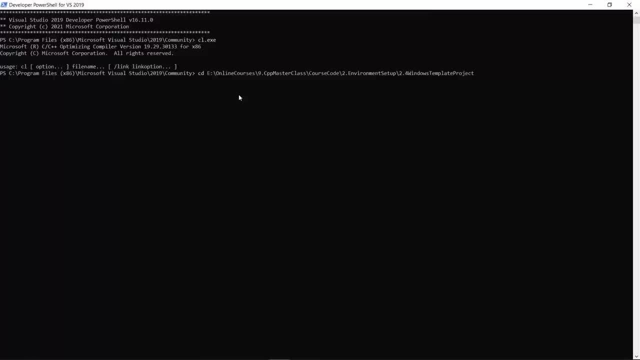 And I am going to change to the location of my project here. So I am going to say cd and paste in the path I just copied And if I hit enter this is going to change to my location. And I really recommend using PowerShell if you have access to this, because it is a little more convenient to use. 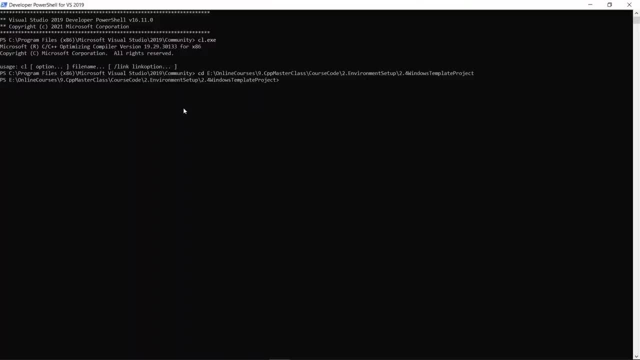 It supports more commands than you can use in the command prompt, But again, that's going to be your choice. Now I am in the location for my project. If I do ls or dir, you can see that. I can see my main CPP file. 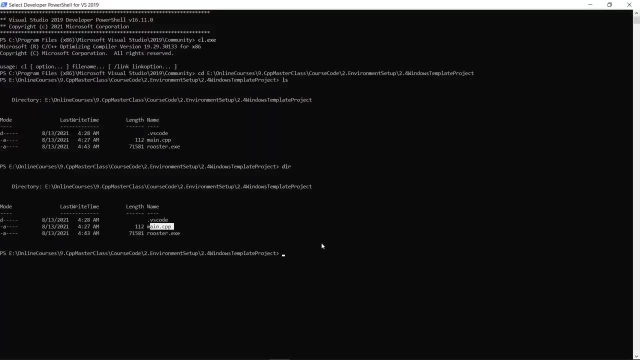 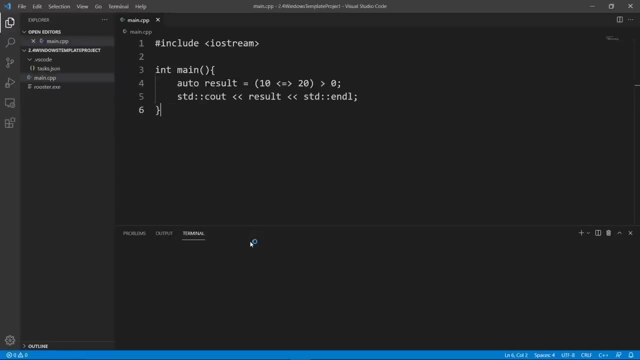 I can see the binary we generated earlier, But this is not a problem. So what I can do here is say code and say a dot, And this is going to start Visual Studio code in the current folder of our project here. So if you hit enter, we're going to wait for Visual Studio code to come up. 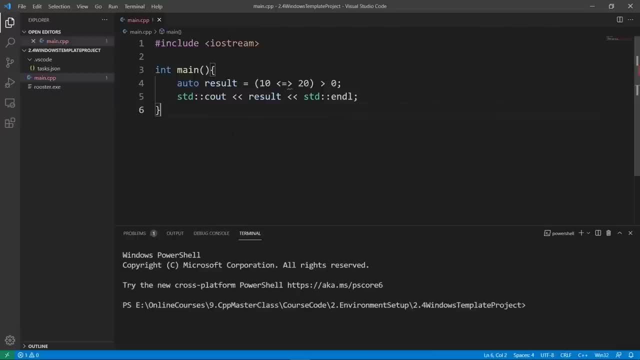 It is going to come up with the project we had in that folder, And the special thing about starting Visual Studio code this way is that it's going to know about the compiler from Microsoft If we come back to our terminal here and clear and say clexe. 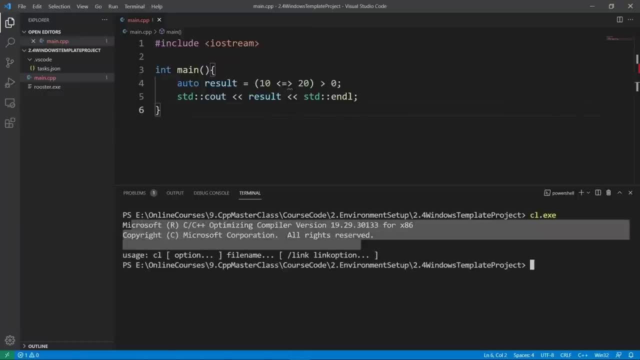 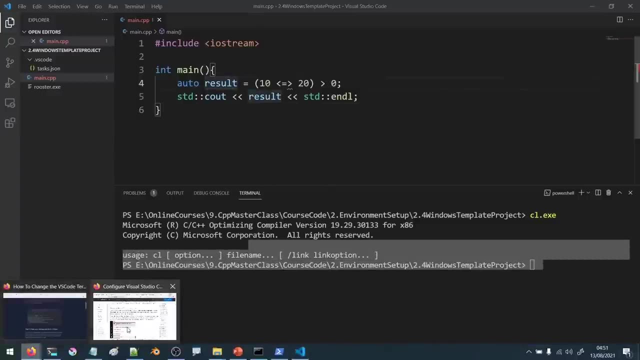 you're going to see that now it knows about the compiler from Microsoft And we can use it to do things. So let's set this up again. If you want, you can read up on how to do this on the documentation from Visual Studio code itself. 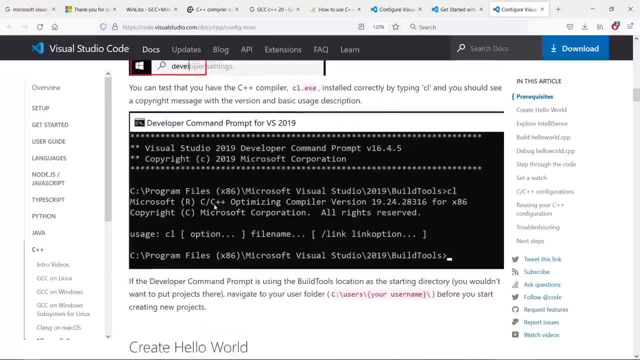 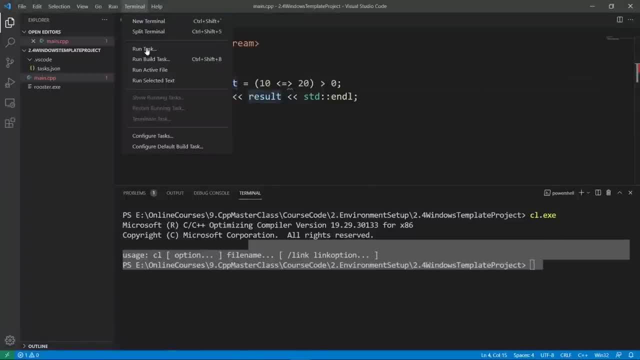 But again, I am going to show you how to do this. You can see that it is really the same things they are doing here. So let's come back to Visual Studio code And we're going to go to terminal And we want to configure a task. 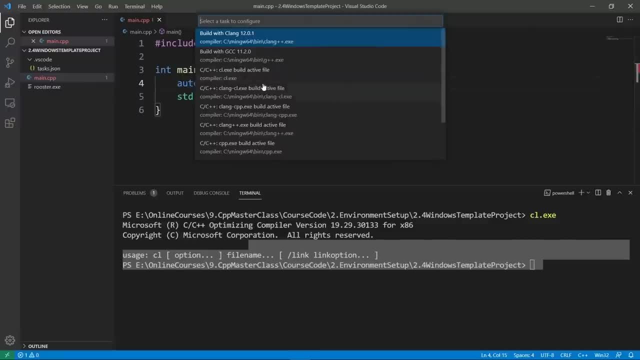 Now you see that we have the compiler from Microsoft available, You can see that we can use that right here. So what I am going to do is click on clexe- build active file, And this is going to add a new entry in our configuration file. 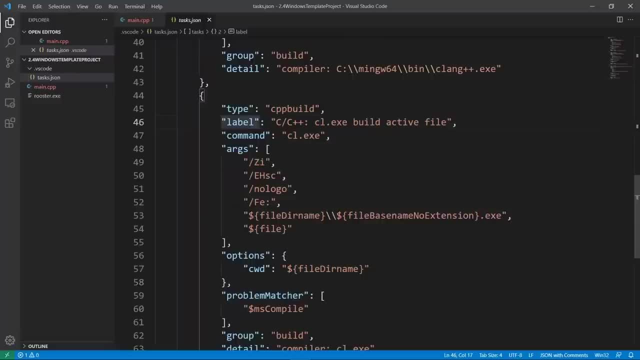 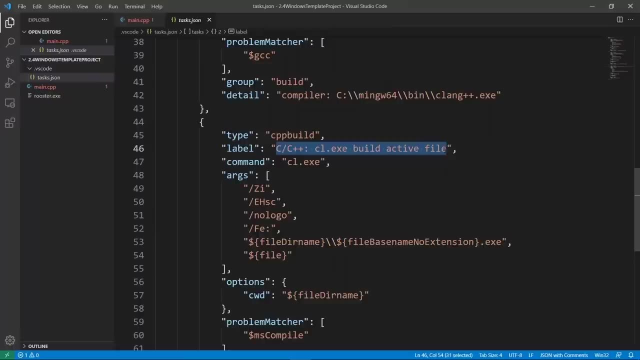 And it is going to open up. If we go here, we're going to find that we have a command to build using the compiler from Microsoft. So let's change the level here And say: build with MSVC. I think this is going to be more descriptive. 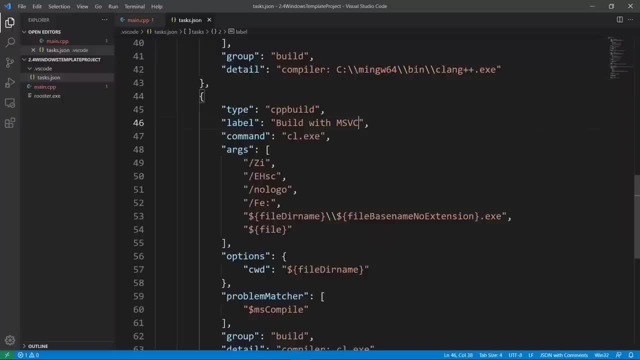 And this is really going to build your thing. Now I am going to change this up so that it builds everything in the current folder And again I am going to remove everything here and put in a configuration that I have ready on my system here. 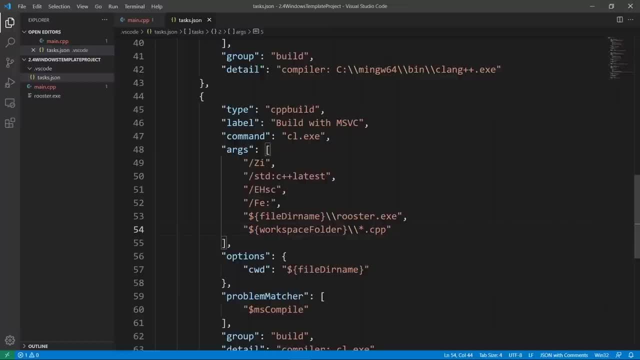 This is what I use for all my projects. Again, this is just calling the compiler and giving it options to do things. We just need to specify this: We want to use the latest standard of the C++ standard And it is going to specify the input files. 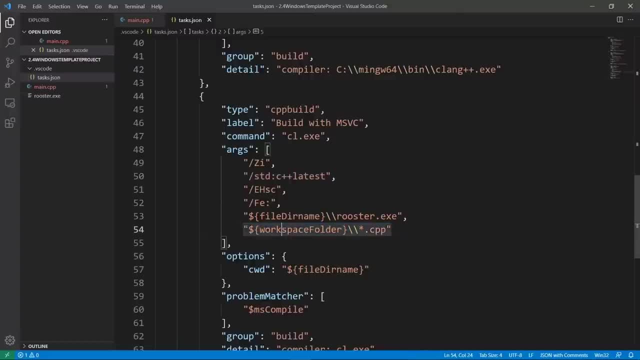 We're going to be building everything in the current folder. This is what we are saying here, And the output file is going to be called roosterexe. If we save this by saying ctrl s or command s and close our tasksjson file. 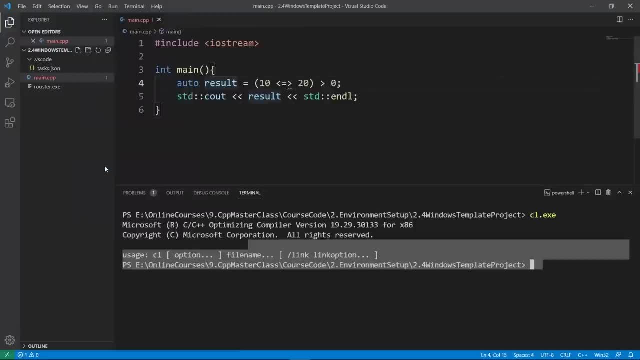 we can bring up our terminal window by going to view and saying terminal here And we can go down and clear. We can say clear and hit enter And if we do rm and say rooster and hit tab, this is going to remove the binary we generated with the Clang LLVM compiler earlier. 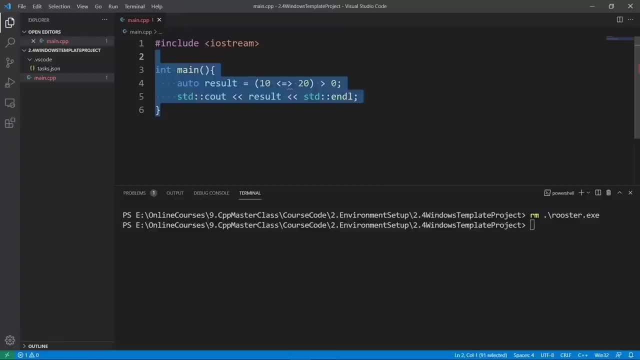 Now we want to build with the compiler from Microsoft, So let's do this. We're going to say terminal And we're going to say that we want to run a task, But this time we want to build with msvc. This is what we want to do here. 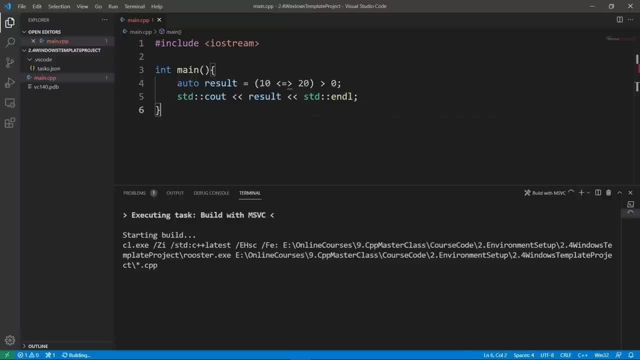 If we click on this little thing, we're going to kick off the process to build with the compiler from Microsoft And we're going to wait for the compiler to do its thing. And if we wait, we're going to see that the build finished successfully. 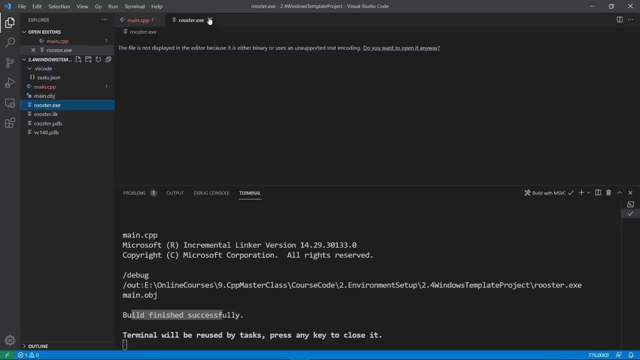 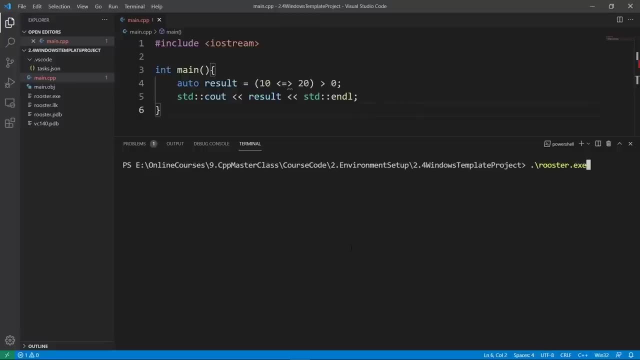 And if we look in our folder, we're going to see that we have our output file And we can come in our terminal and hit enter And do clear, to clear things up. And if we say rooster, just like this, and hit enter. 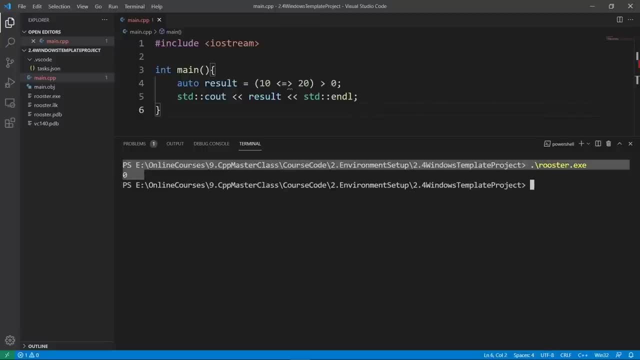 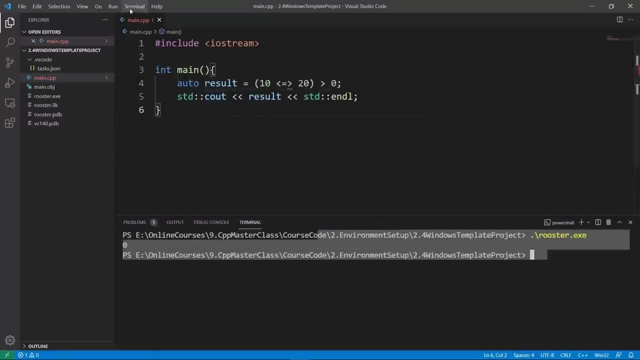 you're going to see that it's going to say zero, And this is confirmation that we are able to use our Visual Studio Code editor and be able to use it with all kinds of crazy compilers, And this is really cool. If you are on Windows, I recommend setting this up. 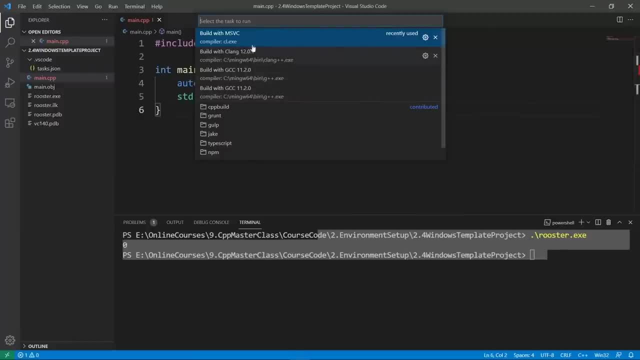 because it's going to make it easier to run C++ applications from Visual Studio Code using state of the art compilers like msvc, Clang and GCC here, And this is really cool. Now we have everything we need to start running C++ applications. 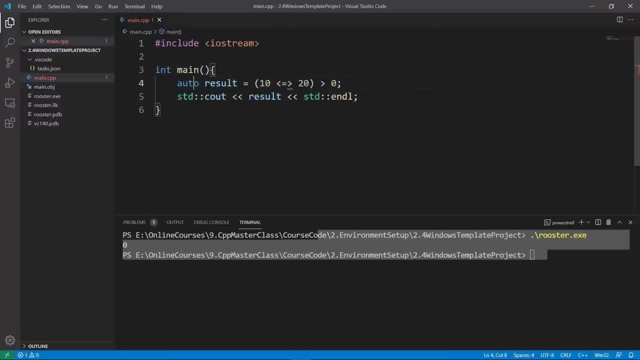 But before I let you go, let's show you how you can set this up so that you have an easier time with regards to IntelliSense and whatever. So what we're going to do, we're going to go to our view menu and we're going to choose command palette. 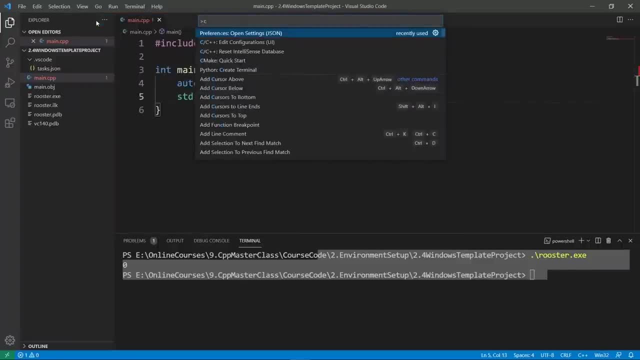 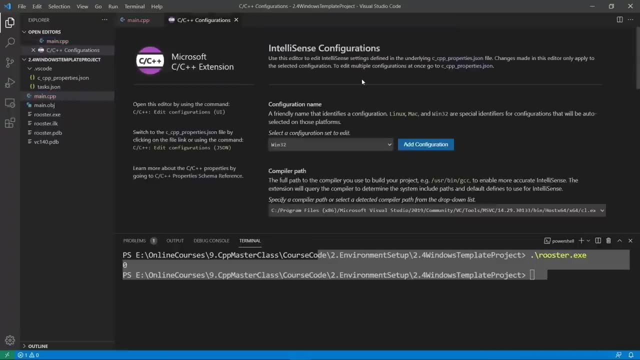 And in this we're going to say C or C++, We can say something like this, And we're going to choose edit configuration UI. This is going to give us an option to configure things, And I want you to configure things in your system. 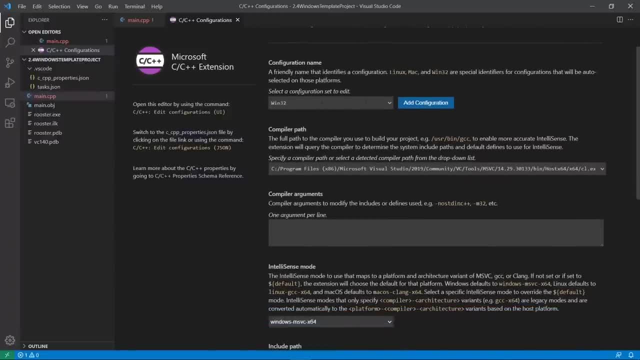 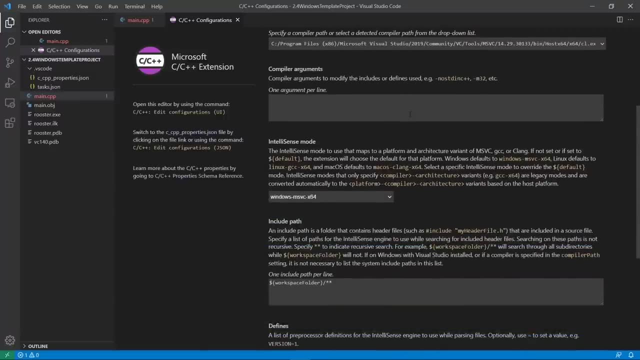 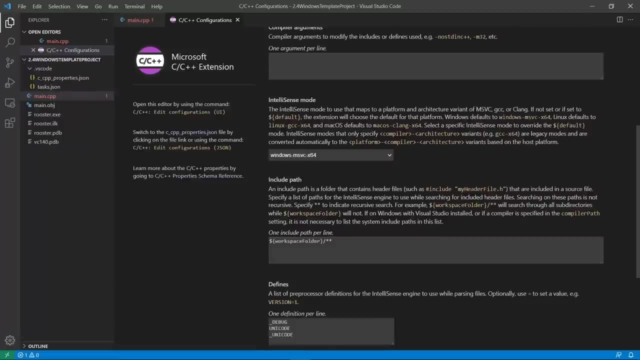 So I am on a Windows system. Let's see the options we have here. I am only going to have the option for Win32. But if we go down we can specify the things we need Visual Studio Code configured for. For example, it's going to give us IntelliSense or autocomplete. 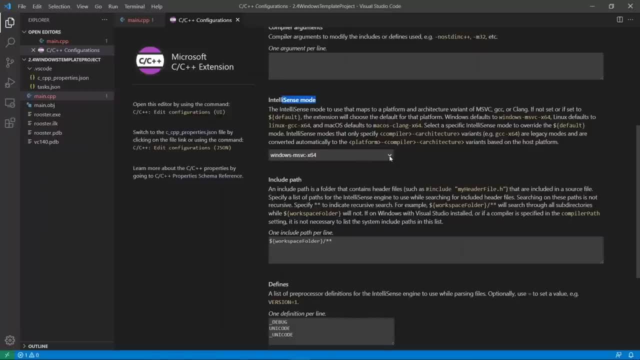 and all kinds of crazy things Using the setting we choose here. if we want, we can choose the GCC compiler or whatever. I am just going to leave in the Windows MSVC compiler because I am on Windows here But know that you can configure these things. 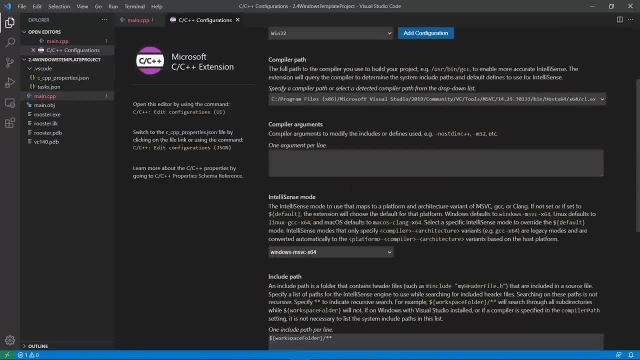 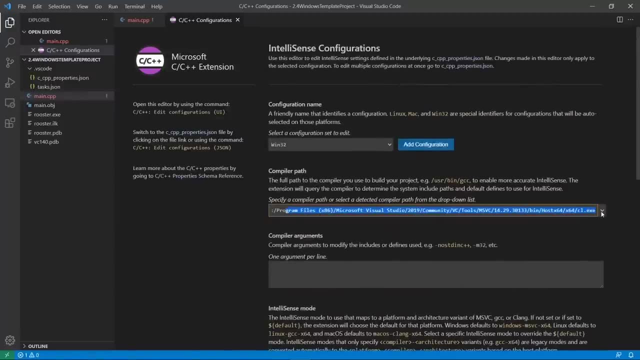 Now, if we go down, we're going to see that we have the option to configure the C++ standard and the compiler path that is going to be used to figure things out. We're going to be using the compiler from Microsoft here, But know that you have the option to choose any other compiler. 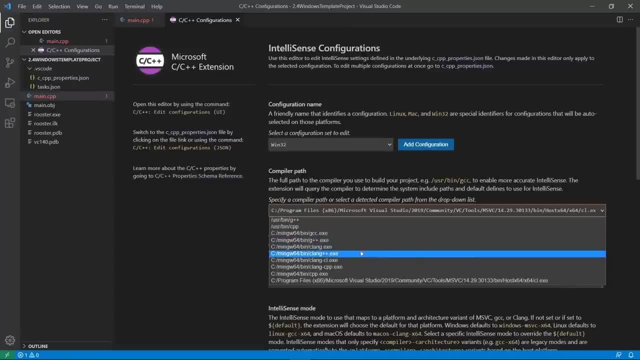 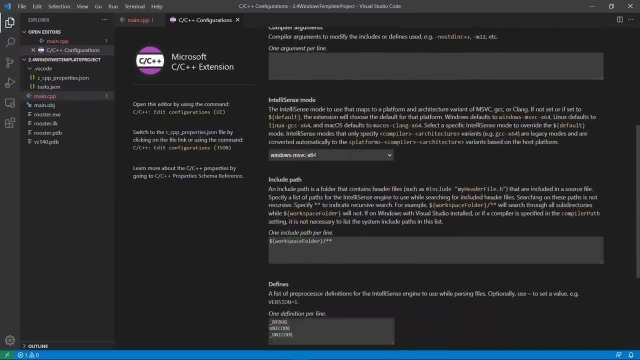 For example, we can choose the G++ compiler, We can choose the Clang++ compiler. You can configure these things And if you need to change this, please come back here and do these configurations here. We're going to leave in this for IntelliSense. 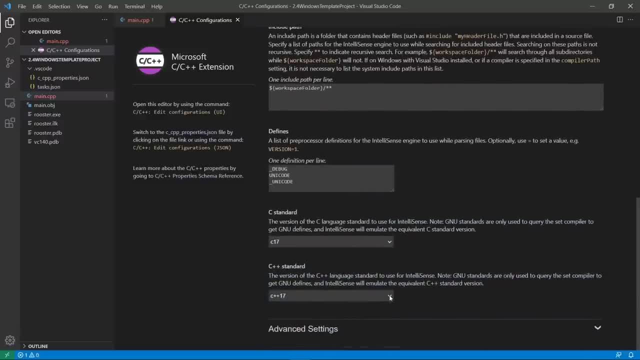 And what we will do is configure Visual Studio Code to use the C++ 20 standard. So we're going to do that right here And if you set this up, you're going to see that Visual Studio Code is going to generate a CPP properties file. 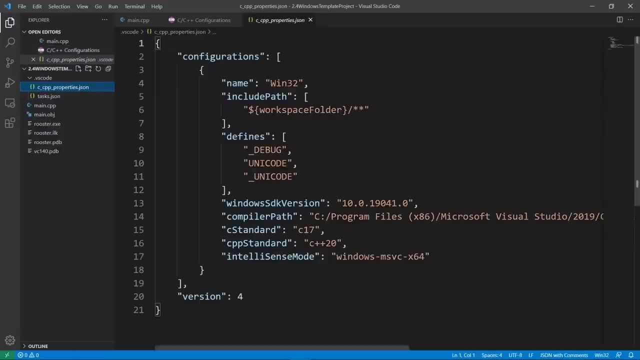 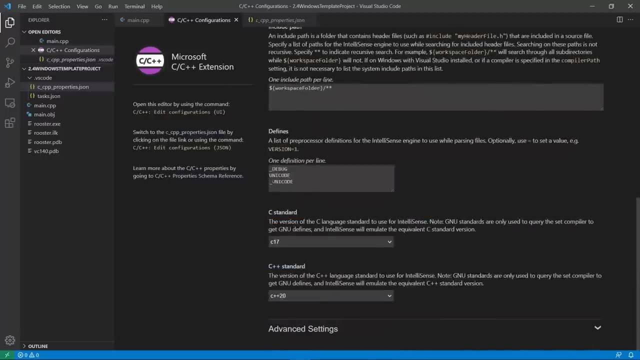 which is going to store all these configurations here. So it is really going to be a configuration for what we choose in our configuration here. So make sure you choose what makes sense. Again, I would recommend using C++ 20. But if you go on top you can really use any compiler you want. 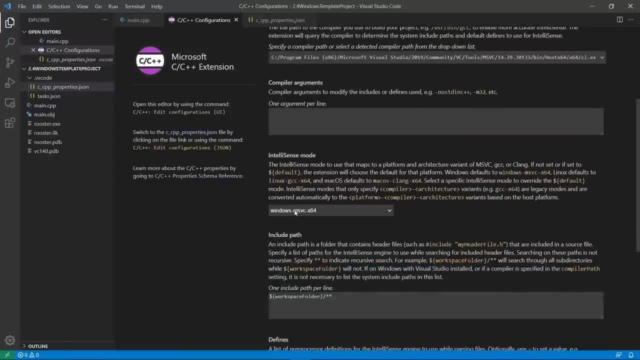 I am going to use the compiler from Microsoft. This is okay. I am going to use Windows MSVC configuration for IntelliSense here And I am going to close this, And we are really ready to start using Visual Studio Code to write C++ application. 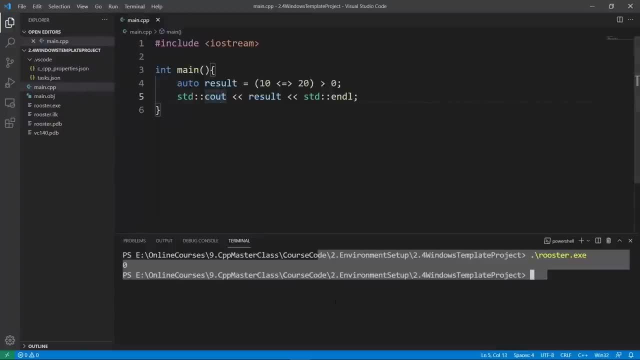 So let's clean this up a little bit. We're going to view our terminal And we're going to remove the junk that was generated by the compiler from Microsoft. I am going to say rm and say rooster, And I can remove the binary. 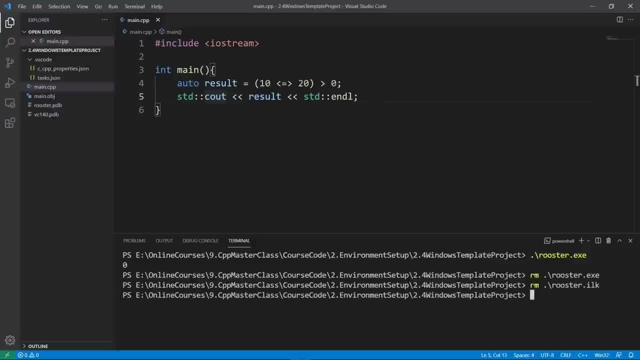 I can say rm and say rooster and say tab. This is going to autocomplete and really remove things I don't need. I am going to remove the PDB file. I am going to remove rooster. I am going to remove the main object file. 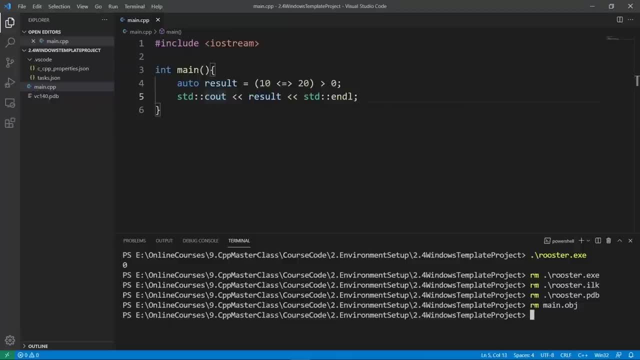 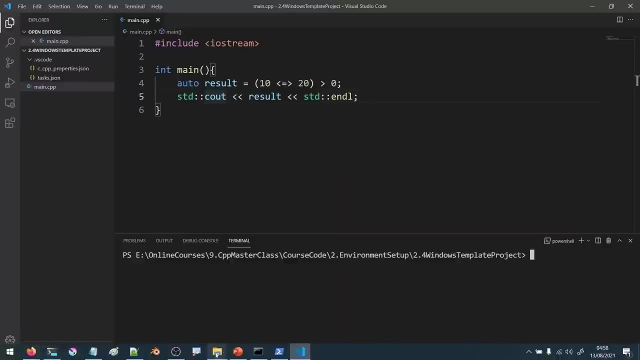 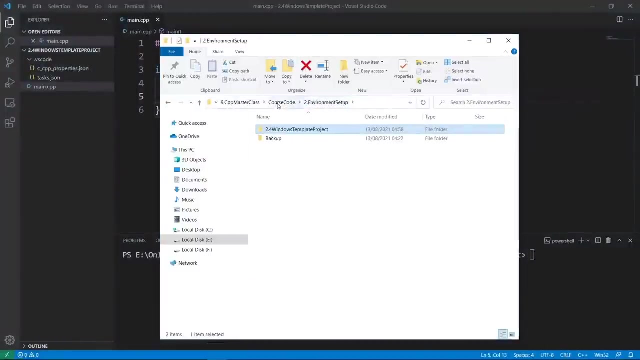 So let's say mainobj And I am going to remove mainorvc, We don't want to remove our CPP file. So now we have a project we can use as a starting point to write C and C++ applications here. So what we will be doing in the next few lectures or the next few chapters is reusing this thing here as a template project. 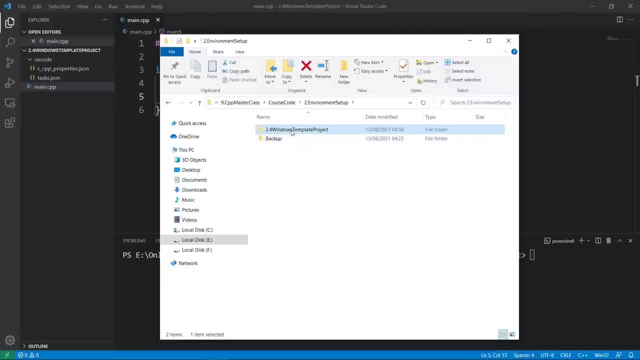 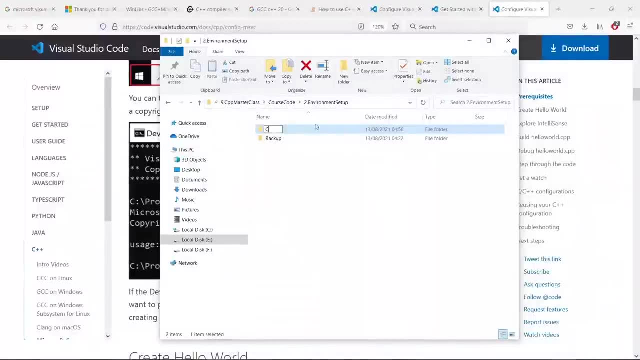 So what I can do is call this C++20 template project, And let's do this here. I think I need to close Visual Studio Code, Otherwise it's going to complain. So I am going to call this little guy C++20 template project. 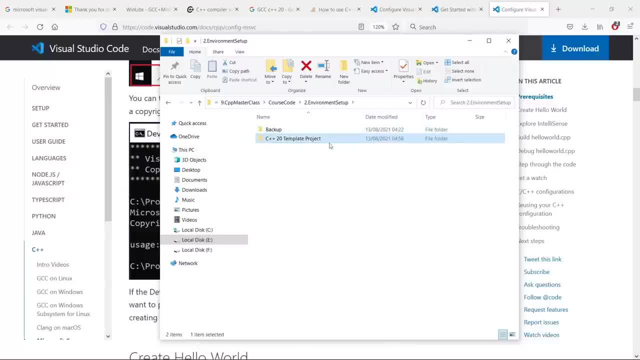 And later, when we start learning about C++ proper. we're going to be using this as a starting point And we won't have to reconfigure the compilers. Our project will be ready to use the compilers that we set up here, Namely the compiler from Microsoft, the G++ compiler and the Clang++ compiler. 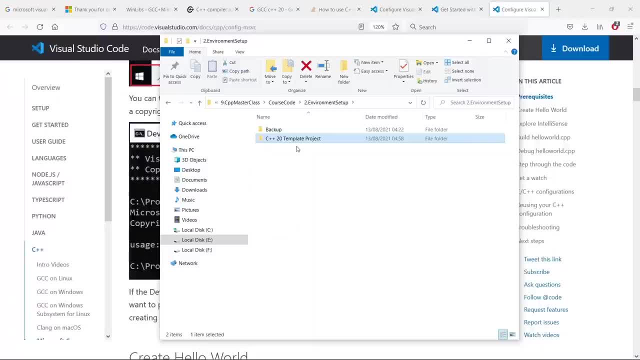 And that's going to be really cool. This is really all I had to share in this lecture. I hope you have Visual Studio Code set up to use all these compilers. We are going to stop here in this lecture. In the next one we're going to start and see how to set up your development environment on Linux. 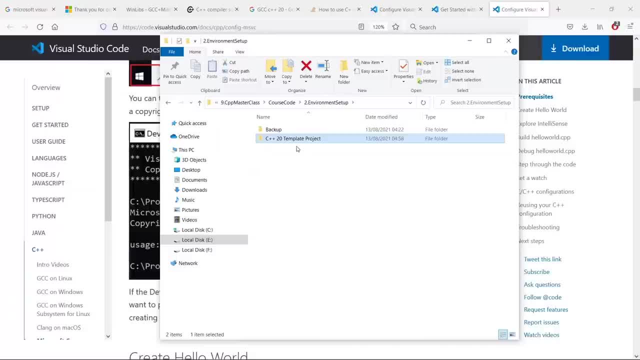 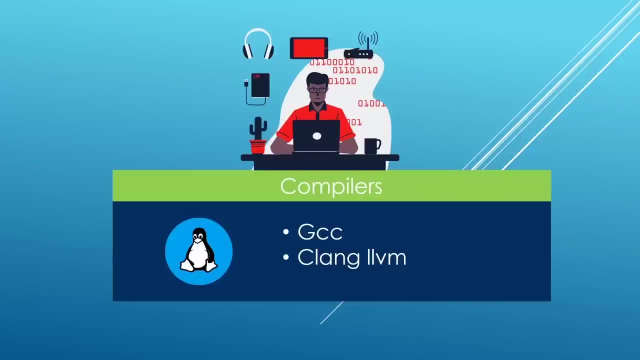 And we're going to start by installing the compilers on Ubuntu 20.04.. Go ahead and finish up here and meet me there. In this lecture, we're going to see how to install C++ compilers on Linux. We are going to be working on an Ubuntu 20.04 system. 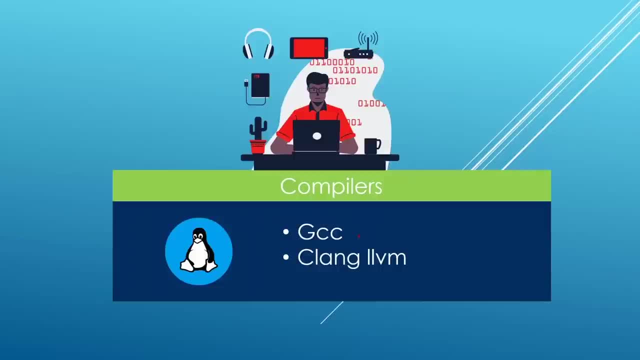 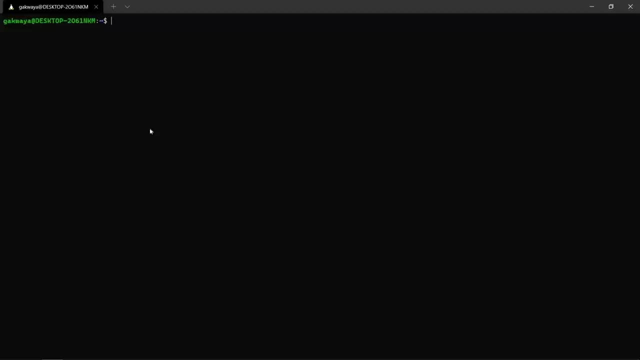 And we will install a new version of GCC And the latest version I can get my hands on for Clang LLVM, So let's do this, Okay. so here I am on my Linux box. This is Ubuntu 20.04.. If I do UNAME and say A, we're going to see the information on this. 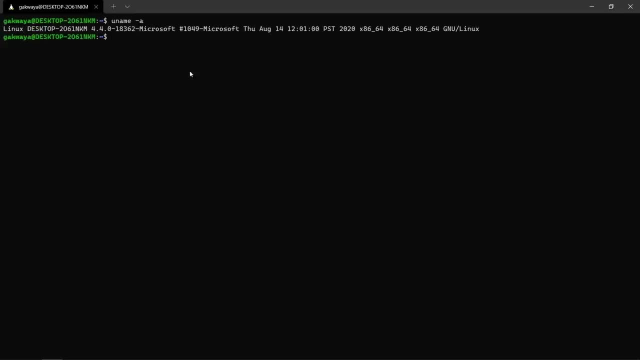 And you will have to adapt this for whatever Linux distribution you are on. And to install GCC, it's really simple. But the problem is the latest version of GCC at the time of recording this video is GCC 11. And it's not available in the Ubuntu packages now. 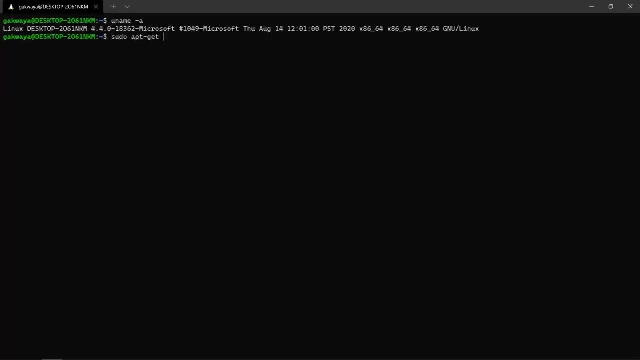 For example, if you do cdu apt-get, install gcc 11.. This is how you get it. If you do this, you're going to put in your password. You're going to see that this is really not available yet, Right. 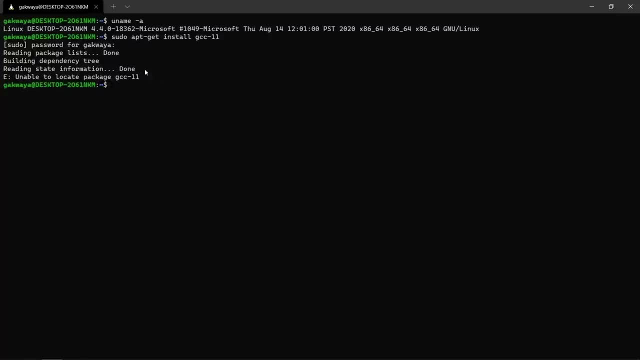 We cannot find this, So the best version we can install is GCC 10,, which I happen to have installed already on this system. So we're going to do GCC 10.. That's what we're going to install here, And if we do this, we're going to see that this is already available. 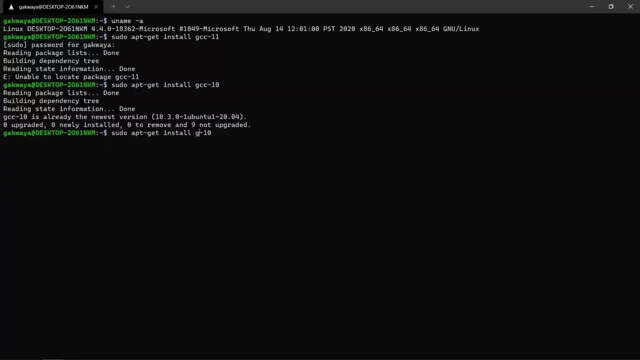 You can also install G++ 10.. I think you can do that. Okay, so we're going to run the command here And we're also going to see that it's already available here. But if you don't have these, they are going to be installed and you can use them on your Linux system. 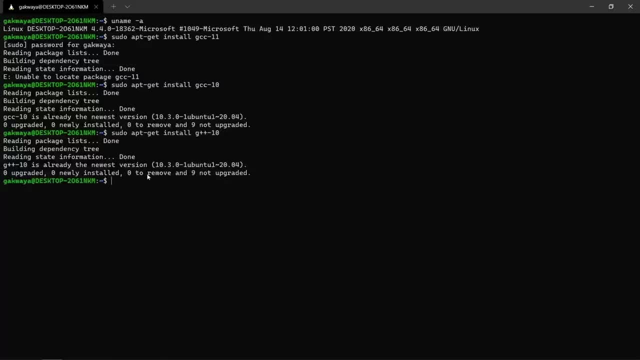 Another tool that is necessary on Linux is the GDB debugger. So we're going to do cdu apt-get install gdb. Right, If you install it, it's going to be installed. But I already have it installed already. So now if I do GCC 10 on my system here and say version. 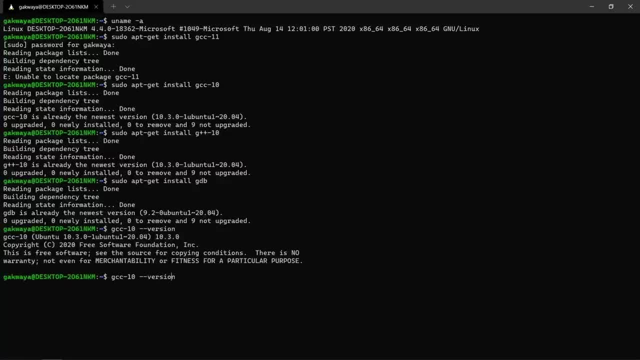 we're going to see the version printed out. We can do G++ 10.. You can see the version here. Let's do that for C++. So we're going to see the version here. We can even do GDB version And it is going to show up. 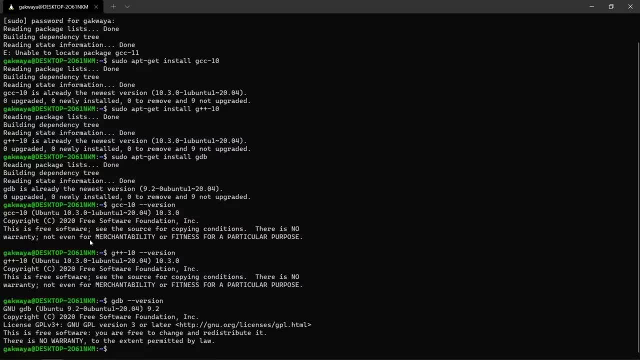 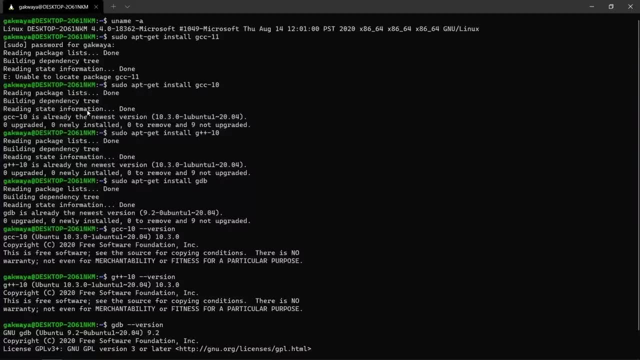 Let's wait for this. We're going to see my GDB version here And now I can use these compilers to compile C++ code on my Linux box here. So this completes our steps to install a GCC compiler on Linux. We're going to look at how we can get a hold. 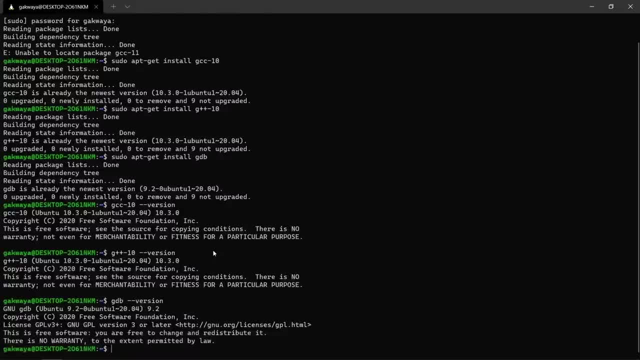 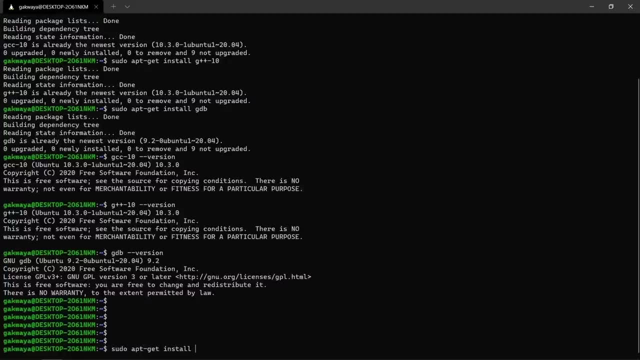 of the Clang compiler on our Linux box here, And it is really simple. All you have to do is to do apt-get install, And we're going to install Clang 12, because that's the latest version at the time of recording this video. 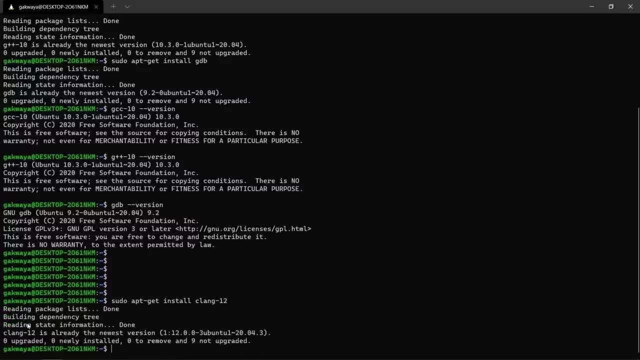 If we do this, we're going to see that it's going to install. I already have it installed here, But if you don't have it installed, it's going to install on your system And this is going to give you all the tools you need to compile. 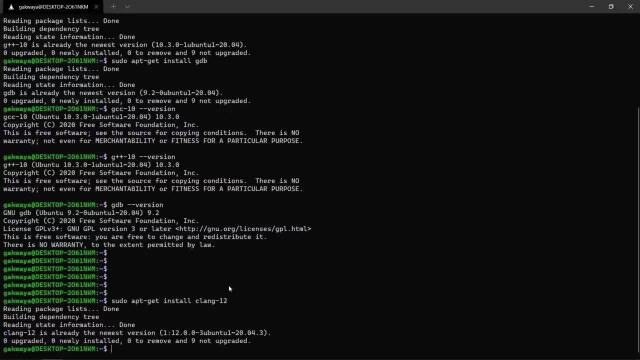 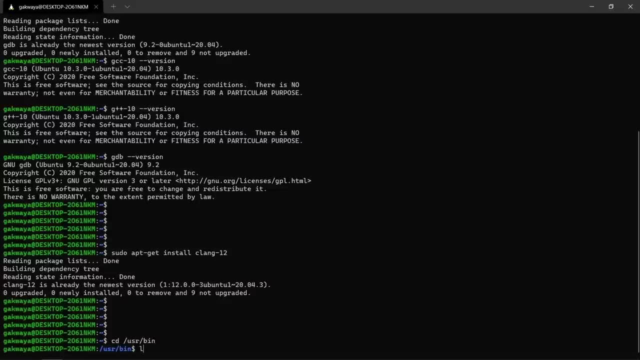 with the Clang compiler On this particular Ubuntu system. these installs are going to be installed in my user bin directory So if I cd there and do analysis to show everything in here And scroll up, We're going to find all the versions for Clang. 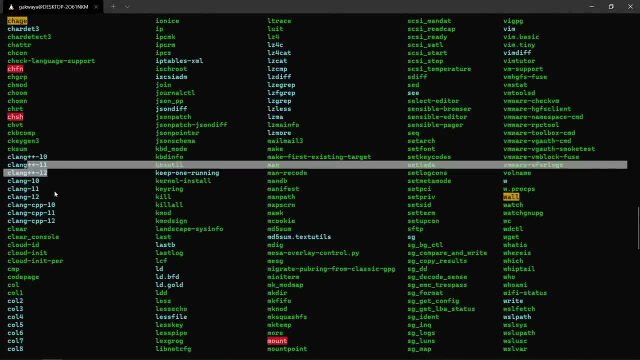 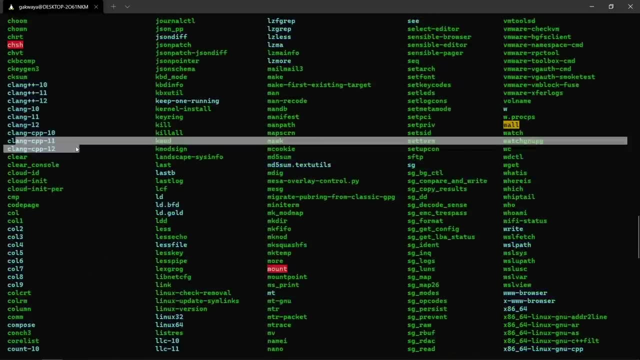 You see, I have multiple versions: Clang 10,, 11, 12.. And we have Clang++ variants of this. I think we do. Okay, we have Clang++ and Clang here And this is going to do what we want. 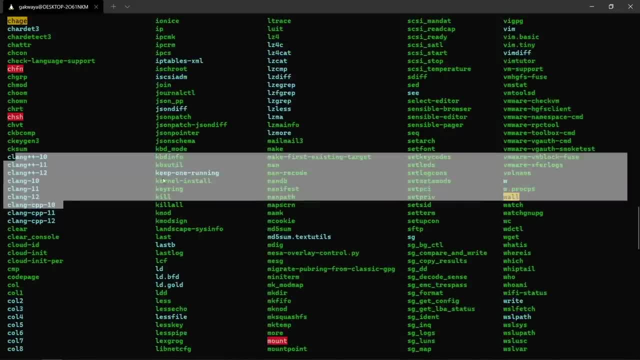 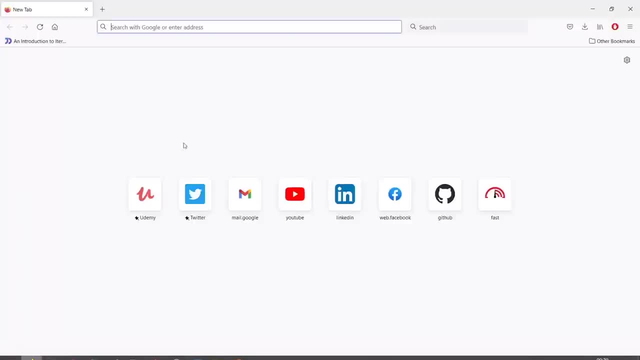 We have the Clang compiler And the GCC compiler installed on our system here Now. if you want to get the latest version of GCC installed on your system, one easy way I found is to go through a package manager called Homebrew. Let's search for this. 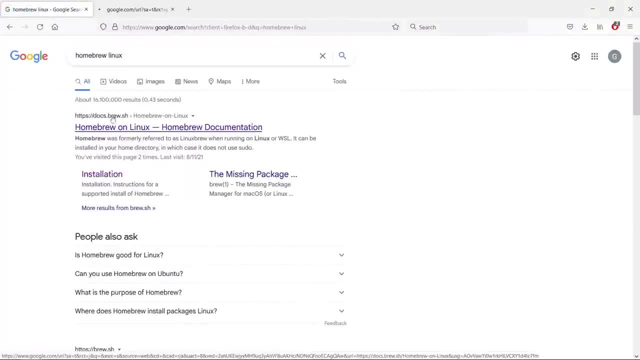 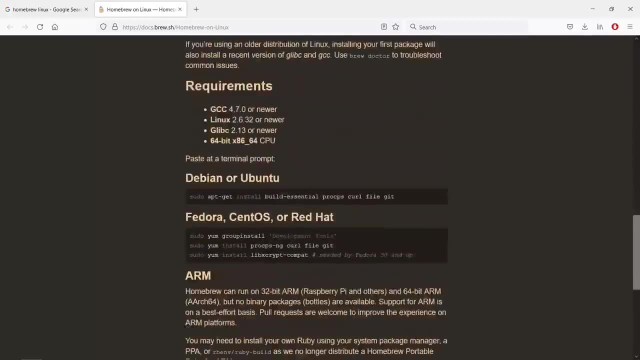 Right, If you search for this, you're going to find it And if you want, you can install it on your Linux system And when you install it, it's going to be basically there, ready to use And to install it. I think there's a command there. 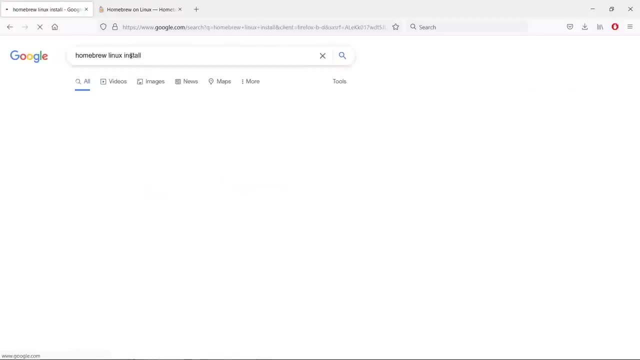 Install Homebrew. Let's do this, Install here. And if we do install, we should find a link to install this. Let's find a link. I think they have a link you can copy. Uh-huh, It is this little thing here. 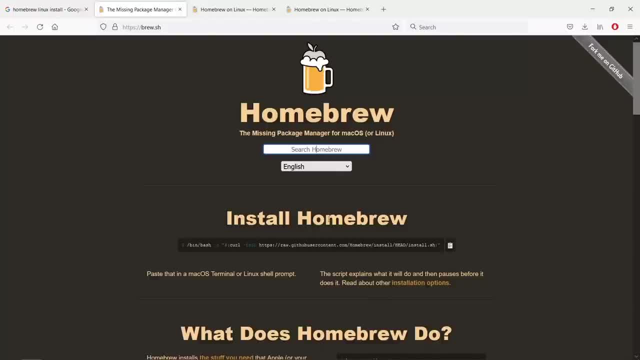 You can copy it, paste it in your terminal and it is going to install Homebrew on your system. And when you have Homebrew installed you can go through it to install the latest version of GCC. For example, if we search for Homebrew GCC in our search engine. 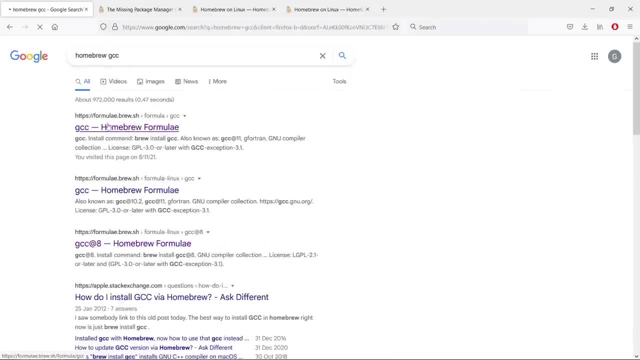 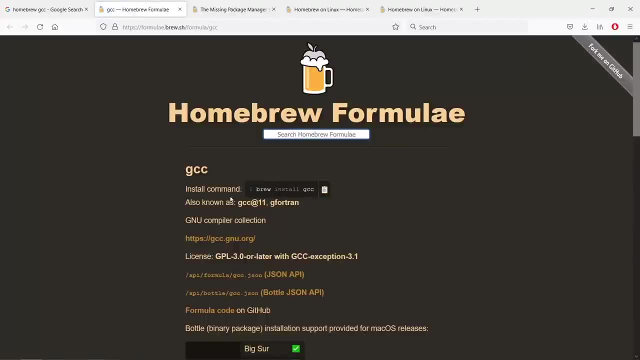 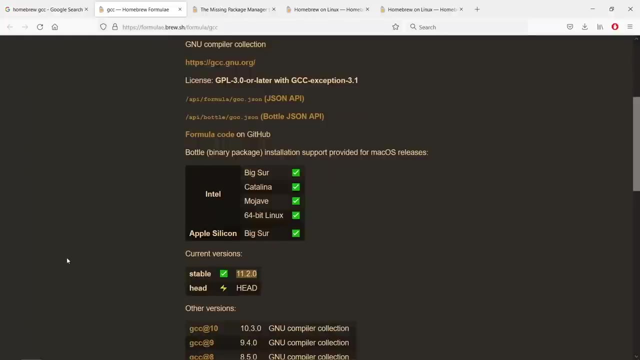 we're going to find all the information to install this through Homebrew And you just have to do brew, install GCC And this is going to install this on your system And you're going to see that it is going to install the latest version after the time of recording this video. 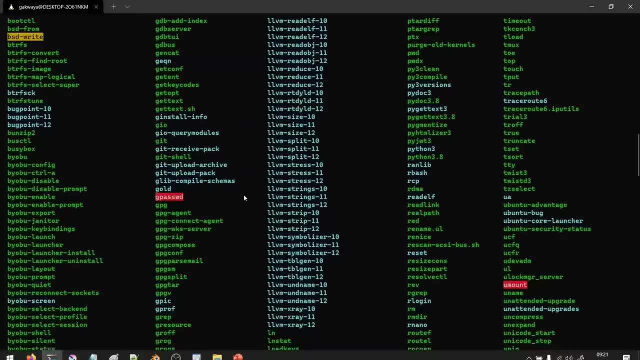 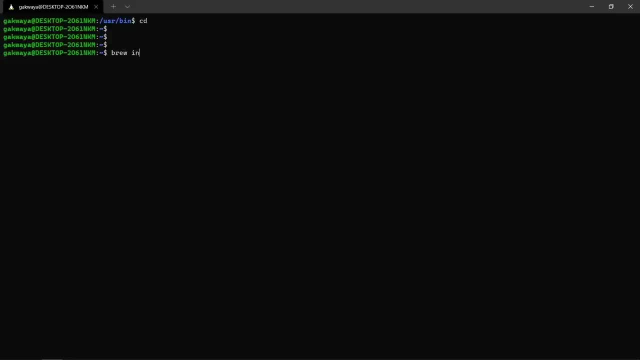 So this is what you should do. For example, if we go back to our Linux box, we can do: let's cd into our home directory And we're going to say brew, install GCC, And it's going to tell me that it is already installed because I installed this. 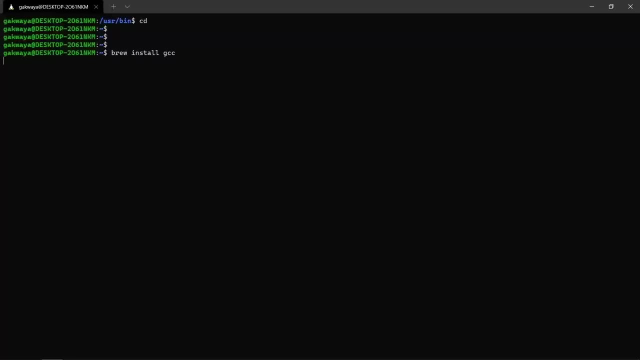 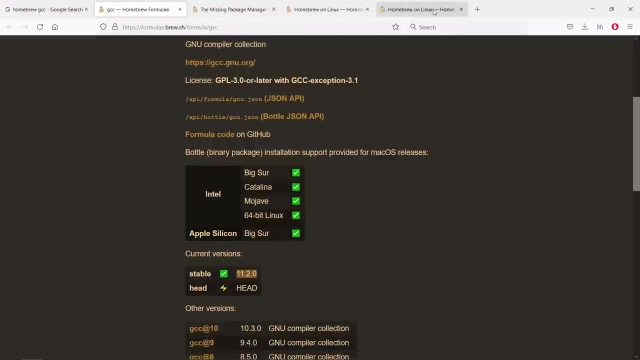 But if you don't have it installed, it's going to install it. And you do this after you have gone through the steps to install the Homebrew package manager on your system. And you do that by just copying this link and pasting that in your terminal and hitting enter. 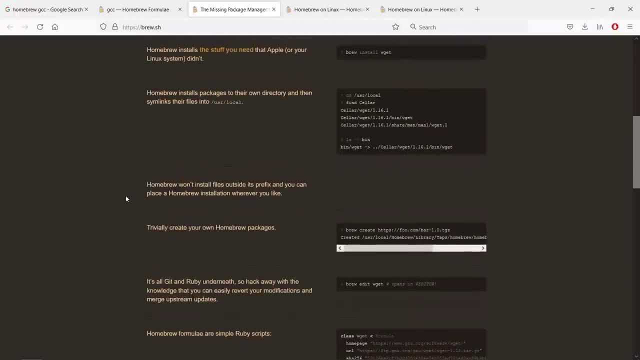 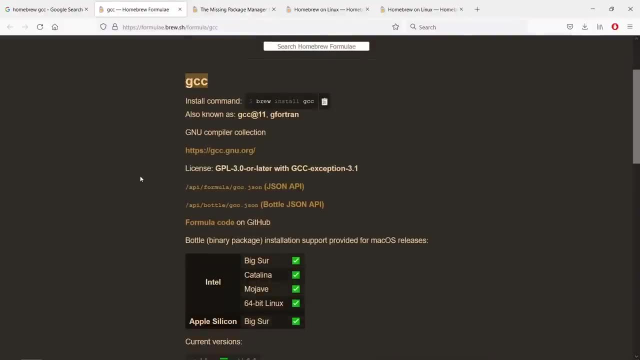 And it's going to give you directions on what you can do to get this properly installed on your system here. So this is really cool. So if you want the absolute latest version in GCC, this is one way you have to get a hold of it. 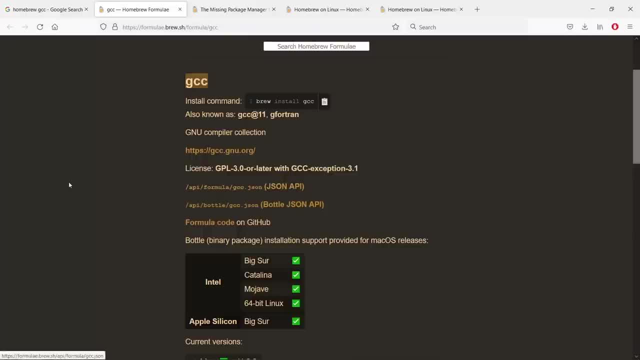 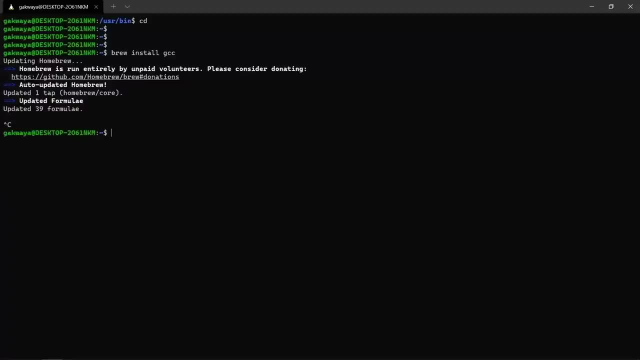 Without really going through the complex steps to build a compiler yourself on Linux. Okay, it is taking some more time here. I am just going to kill this because I already have the latest version of GCC here. If I do GCC 11 on Linux and do version, I am going to see that I have 11 too. 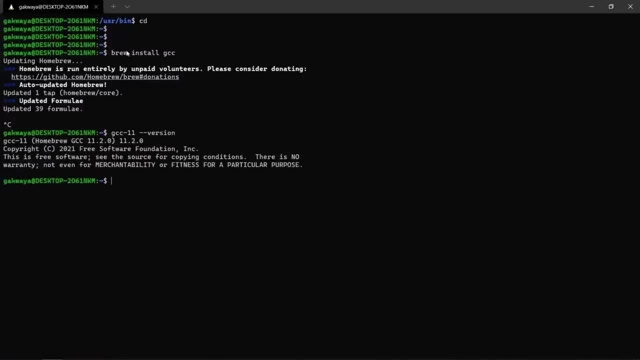 And it was installed through Homebrew, And if you let this run to completion, it's going to install this on your computer. We don't have to wait for this. So now we have the latest version of GCC on an Ubuntu system. We also have the latest version of Clang. 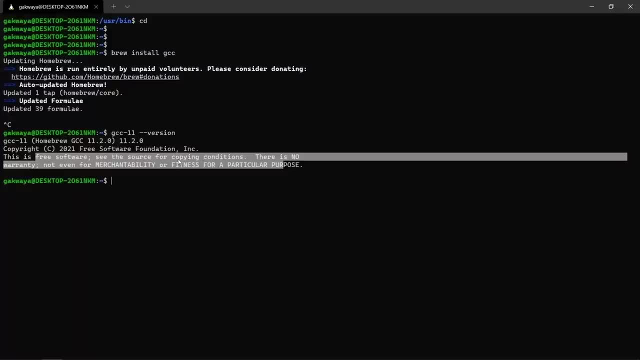 This completes our tutorial on how to set up compilers on Linux. We are going to stop here in this lecture. In this one we are going to install Visual Studio Code on the Linux system, And then in the next one, we are going to link Visual Studio Code to these compilers. 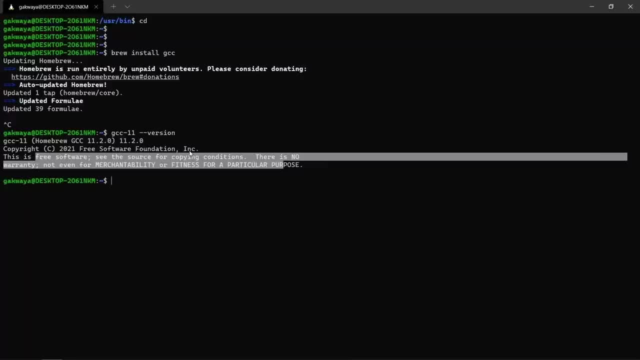 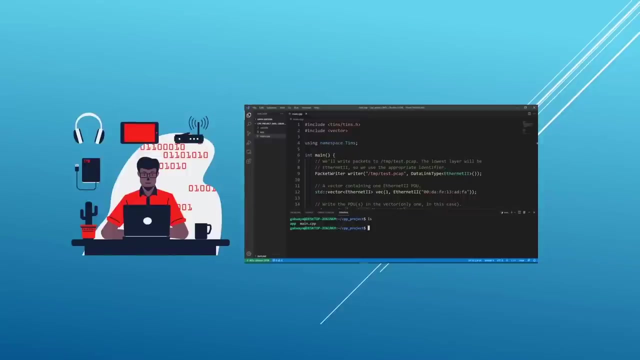 And be able to use them To use Visual Studio Code type code and compile our programs using these two compilers here. So go ahead and finish up here and meet me in the next lecture. In this lecture we are going to see how to install the Visual Studio Code editor on a Linux system. 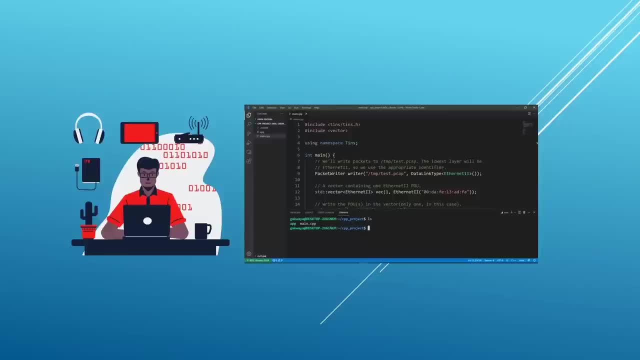 And again, we will be working on our Ubuntu 2004 system here. So let's head over to the website for Visual Studio Code and download our binary And install it on our Linux system here. So here we are at the website for Visual Studio Code. 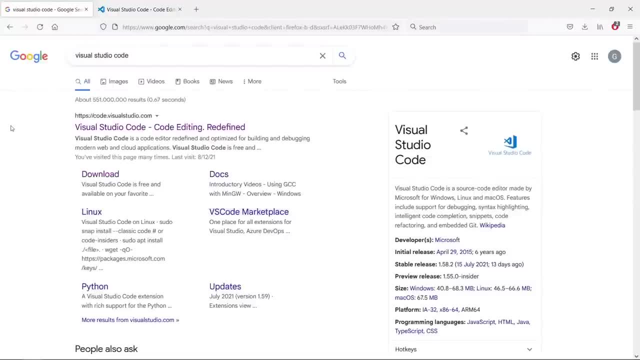 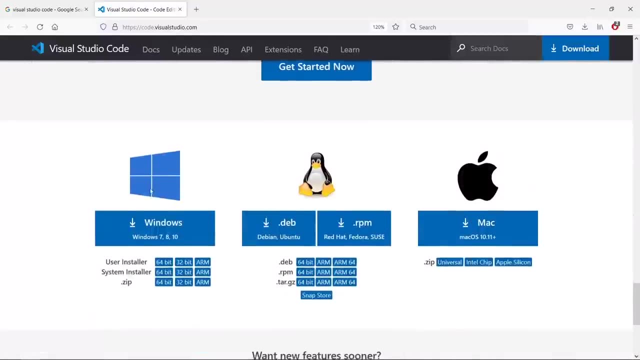 You can get there by searching for Visual Studio Code in your search engine And you are going to land here And all we really have to do is go down to find our download links. We are going to see that for Debian and Ubuntu. we can download here. 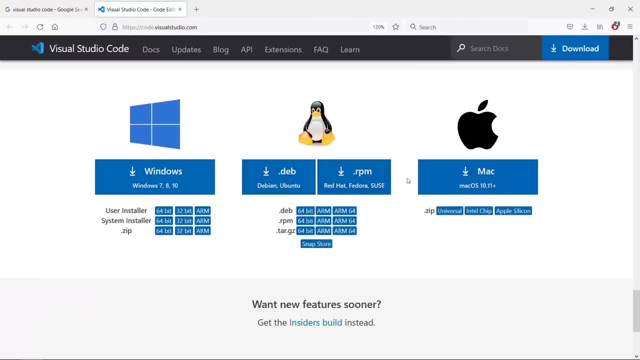 But you can also find something specific to other distribution. So we are going to grab the 64-bit version of Debian and Ubuntu here, Because that's my system And you are going to find whatever makes sense For your distribution. So let's grab this here. 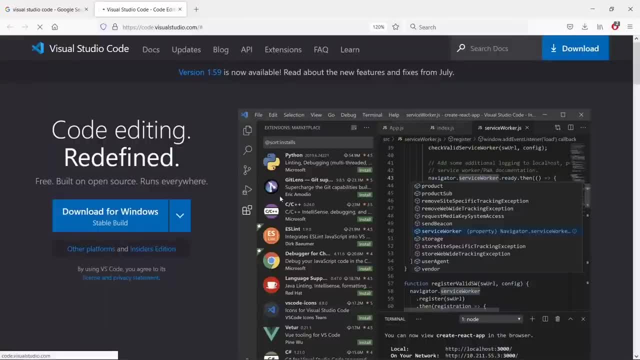 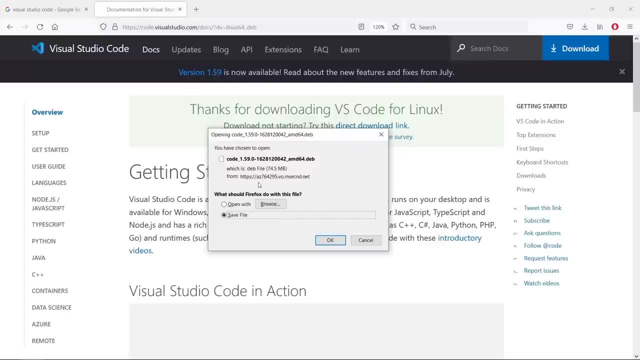 We are going to grab the link. So if you click on this, this is going to kick off the download process And you will see this downloaded on your system. And once you have this downloaded, you are going to install it And in Ubuntu you can just double click on this to install it. 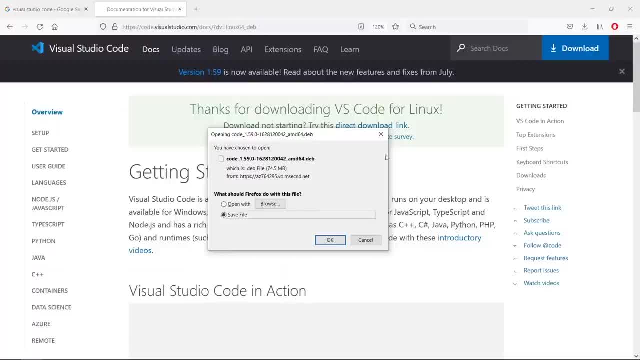 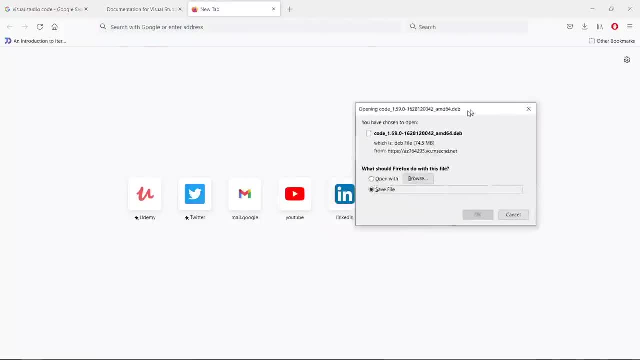 Or you can install it like you install any Debian package on a Linux system, For example. if you are unsure on how to install Debian packages, All you have to do is do a simple search. So let's do googlecom and go there. 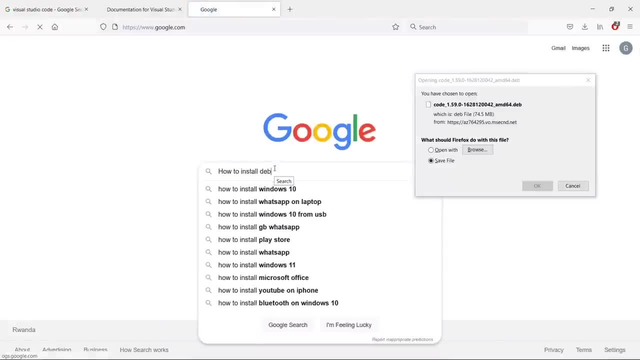 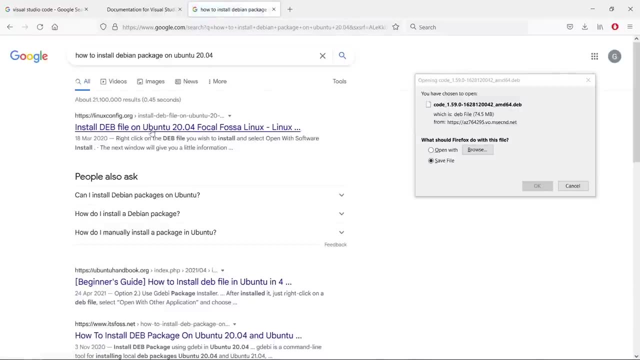 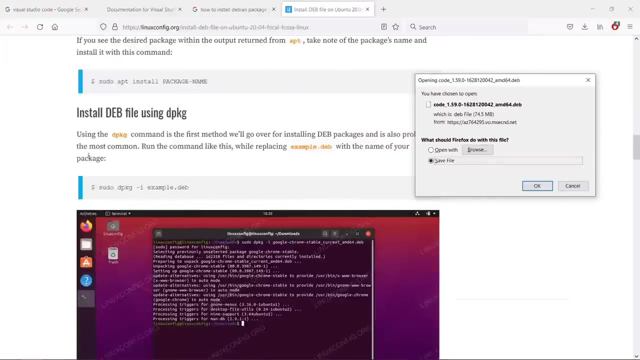 And we are going to see how to install Debian packages on Ubuntu 2004.. So this is our version here, And you are going to find a lot of instructions on how to do this. It's going to be really simple, So we can go down and find a way to install. 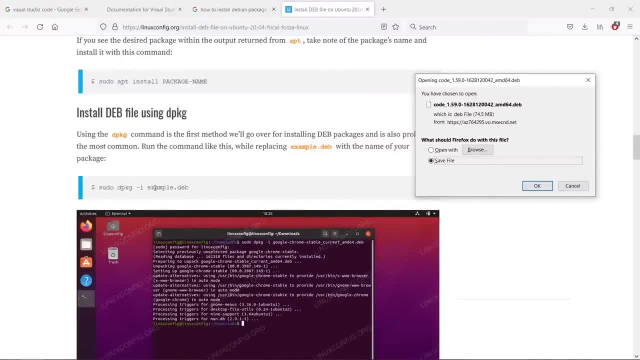 So all you have to do is say to do dpkg, Say I, and pass the name of the package, And this is going to install Visual Studio Code on your system. Once you do this, you will have Visual Studio Code installed And you will be ready to start it and use it on your system here. 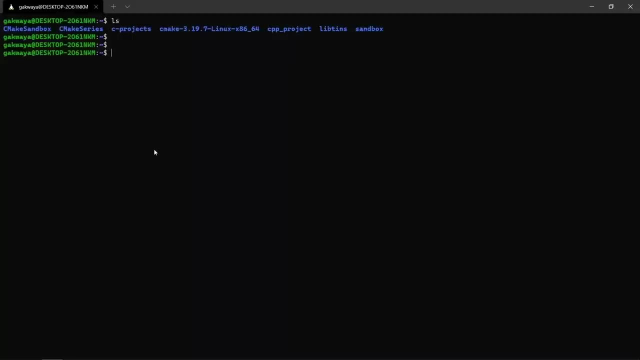 Once it is installed, you will have the ability to come in your system here, For example, and say code dot, And this is going to open a Visual Studio Code instance on your system. Let's wait for this to come up so that you really see this. 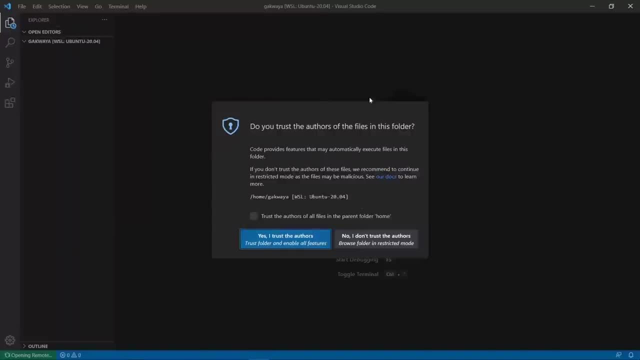 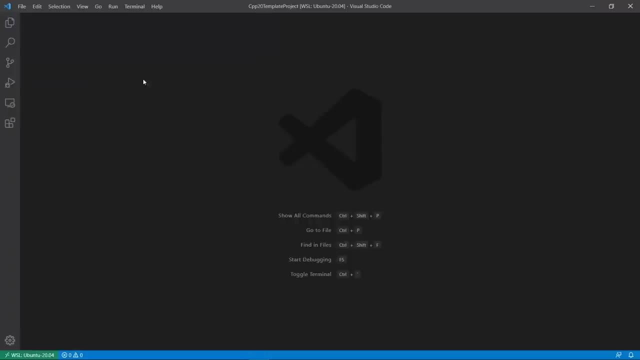 Okay, so this is going to open Visual Studio Code on your system And you can start using it, like we will do in the next lecture. Okay, once you have Visual Studio Code installed and started up on your Linux system, the very first thing you need to do is to install the extension that is going to allow you to do some C and C++. 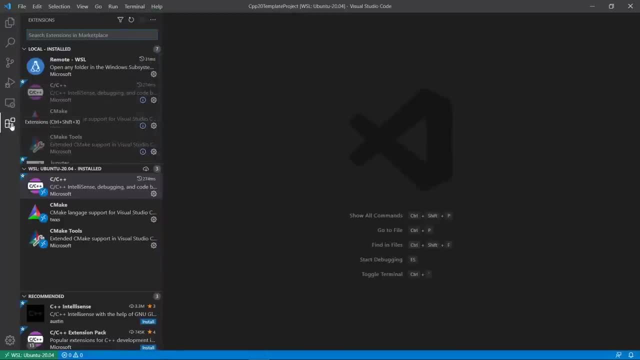 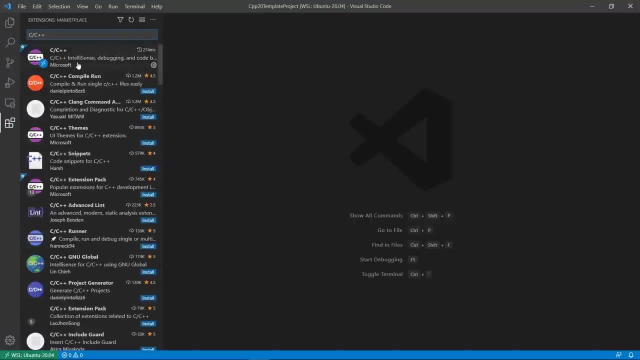 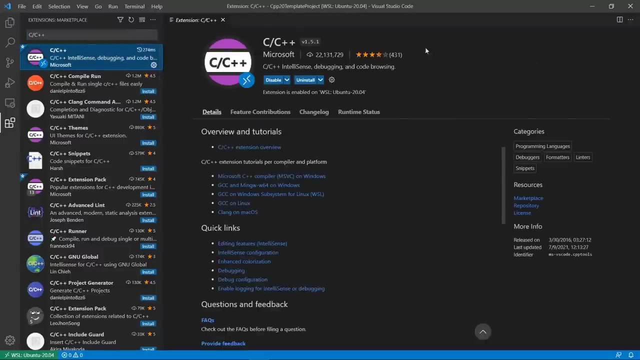 And to do that, you will come to this tab here that says extension, And in our search box you can start typing C and C++ And you are going to have an entry that says Microsoft here, so please select this And this is going to be the extension you need to install. 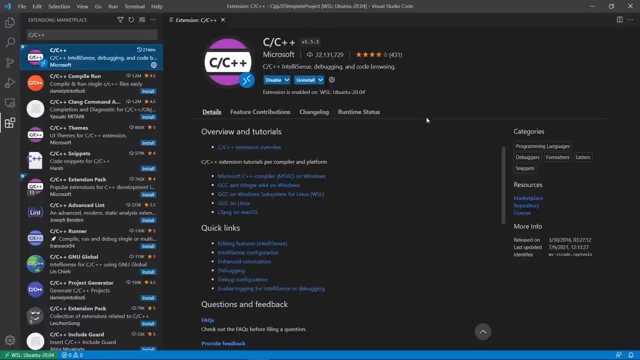 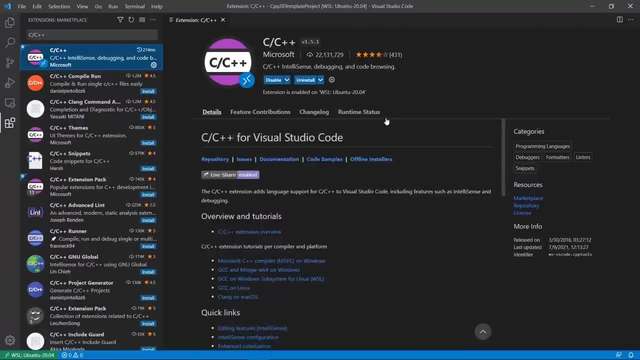 You are going to click on install And it is going to install And this is what enables Visual Studio Code to do some C++ programming And this is really cool. If you want, you can check out how to use it on Linux. 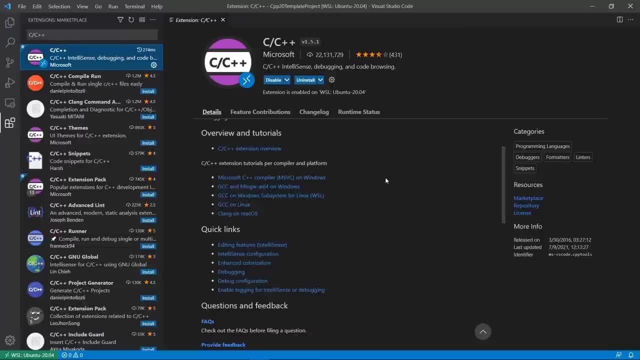 And you are going to have instructions on how to do this, But we will do this in the next lecture and show you how to configure Visual Studio Code to use the compilers that we have installed in a previous lecture. So we are going to tell Visual Studio Code to use our Clang compiler. 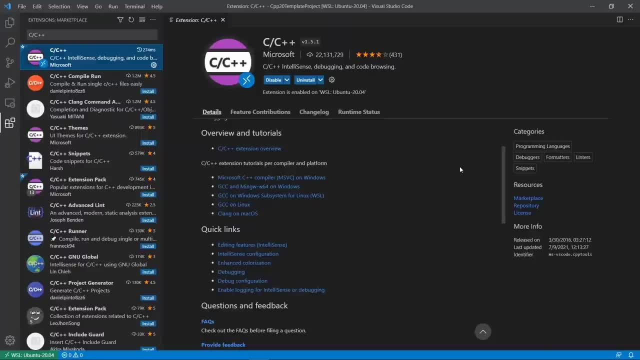 We are going to tell it to use our GCC compiler And we will have the flexibility to come to terminal and choose which compiler we want to use, And we are going to do all this in the next lecture. So go ahead and finish up here and meet me there. 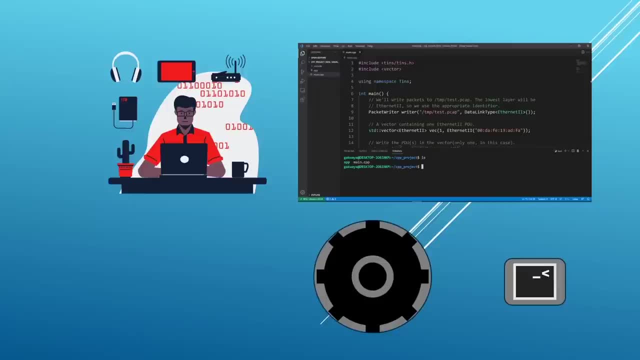 In this lecture we are going to configure our Visual Studio Code editor to use the compilers that we just installed in a few previous lectures. So we will be able to type our code in our Visual Studio Code editor, just like we do here, And we will pass the code through the compiler. 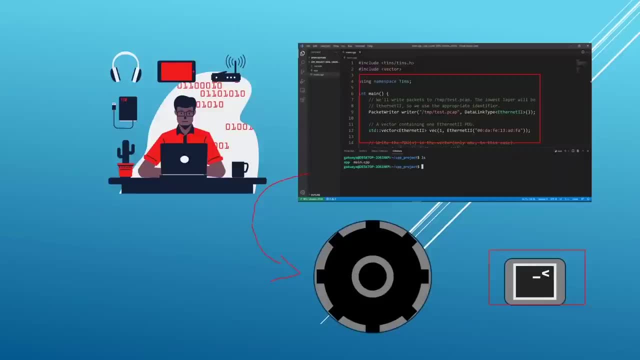 to generate the binary that can, in turn, run on our Linux system. here. This is what we want to do, So we want Visual Studio Code to use the compilers that we installed. So let's head over to our Linux box and do this. Okay, here I am on my Linux box. 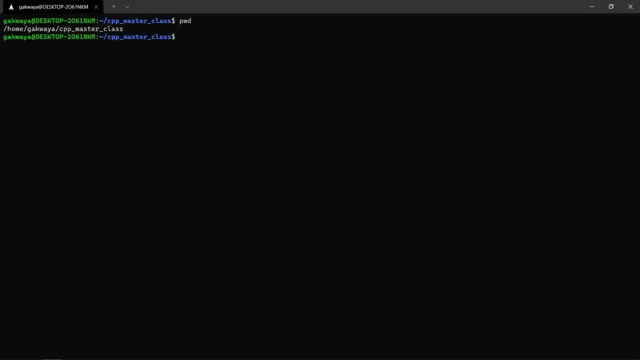 This is the current directory where I am at. This is where I am going to do my things here, So I am going to create a folder and call it a template project. Let's do this. We are going to say mkdir And we are going to say c++20 template project. 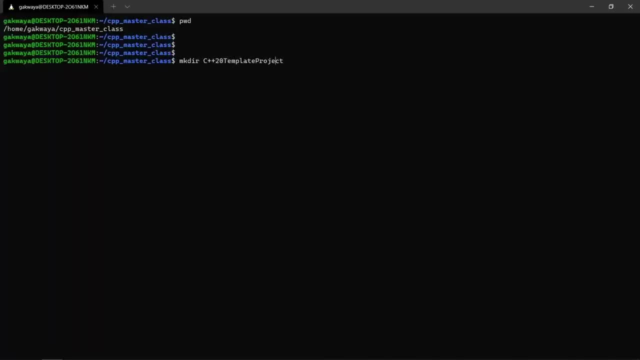 I think this is going to do, Or we can even say cpp, because I am not sure The plus signs here are not going to give us a problem. Let's play it on the safe side And we are going to create this folder. 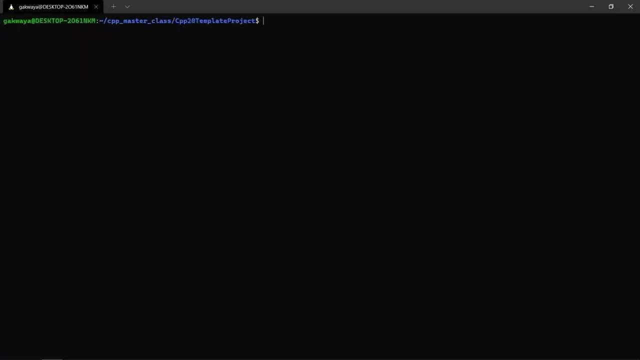 And we are going to cd into this folder. Okay, once we are in this folder, we are going to open this folder in Visual Studio Code, And the easiest way to do that, once you have Visual Studio Code installed, is just to type code and type dot. 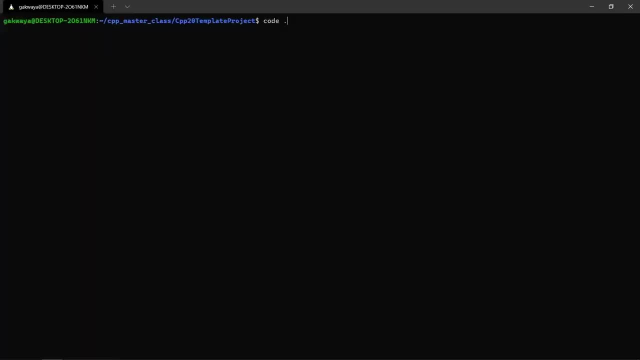 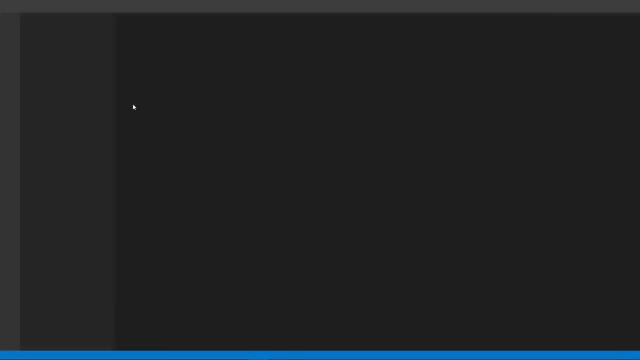 And you will basically be telling the operating system to open Visual Studio Code in the current folder here. So I am going to hit enter And this is going to kick it open. And I trust this folder because I just created it And we are in our project now. 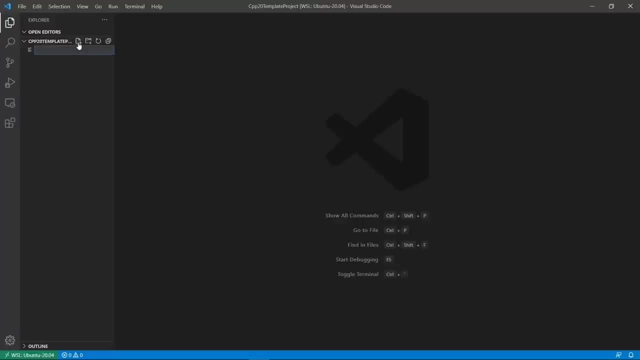 The very first thing we are going to do is to create a main cpp file. So let's do that. And I did that by clicking on the plus icon here And I typed in the name of the file- And I am going to put in some dummy code here- that we want to use our starter code. 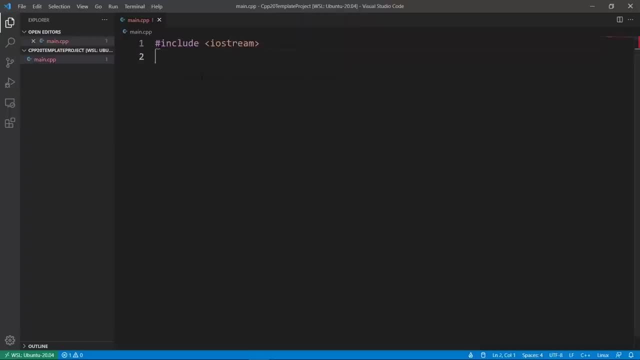 We are going to say iostream And we are going to put in our code here. We are going to say main. And again, you don't have to type all this. If you want, you can get the code from the resource section on the lecture. 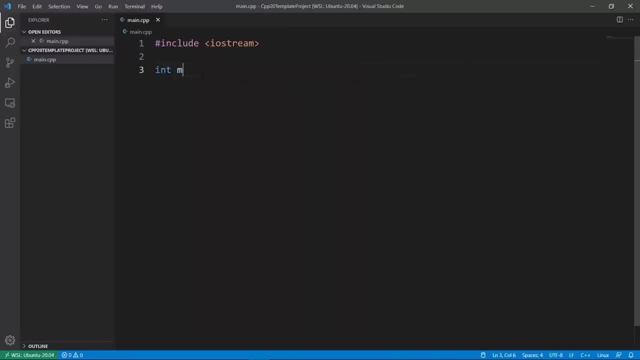 So you can copy the code, paste that in here and be on your merry way, Because we haven't really started learning about C++. we are setting up the environment, So don't stress yourself here. This is just some simple code to test our compilers to see if they support C++20. 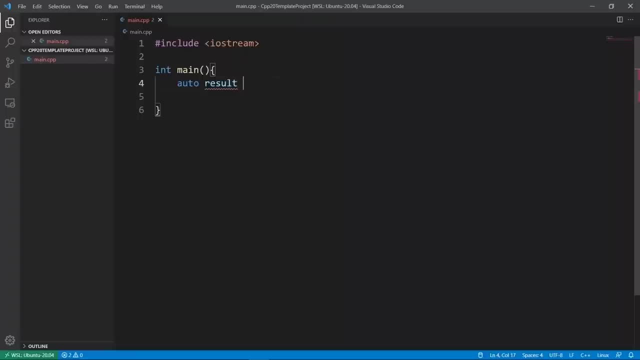 Because we want to use the latest standard we can get our hands on here. So let's do equals Type- exactly what I typed here. So we are going to say 10.. And we are going to put this weird operator and say 20.. 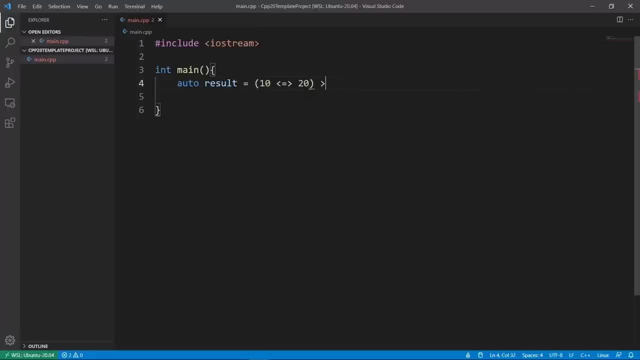 And we want to see if this madness here is greater than 0. This is what we want to do And we are going to say stdcout and say result. So type exactly what I typed here And as we progress in the course, we are going to make sense of all this madness we see here. 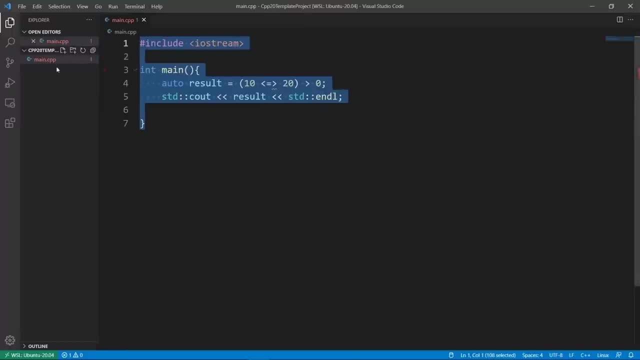 So now that we have a CPP file containing the code for our C++ program, we want to compile this And we need to tell Visual Studio Code which compiler it's going to use to compile this program here to give us a binary that we can run. 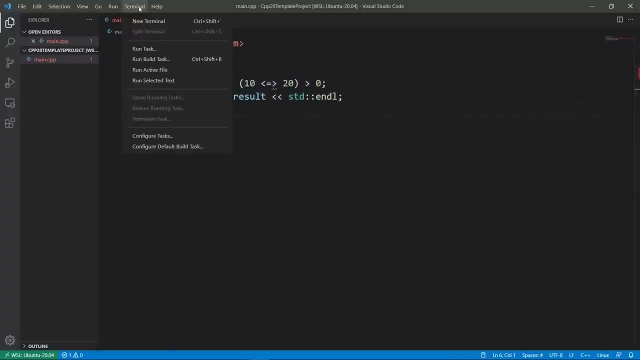 So what we are going to do is come to terminal here And we are going to say that we want to configure tasks, And a task is really a set of instructions you give to Visual Studio Code on how to take your C++ project and turn that into a binary that can run on that system. here 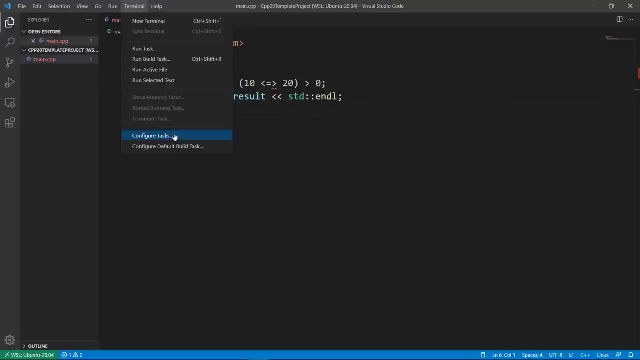 So that's what we want to do. We want to tell Visual Studio Code which compiler it's going to use. We are going to configure tasks here And you are going to see that it's going to discover many compilers on my system here. 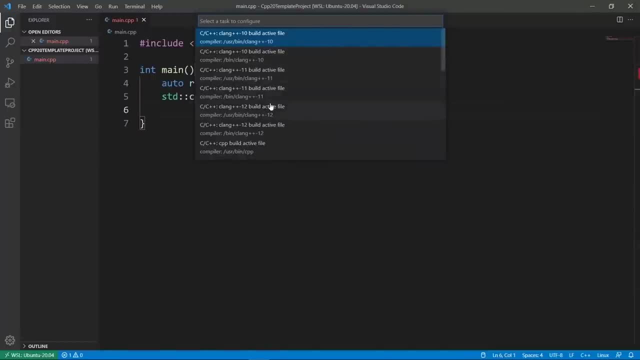 You see we have Clang 10,, Clang 11,, Clang 12.. And we should also have GCC 11.. If we keep scrolling down, we are going to find these little guys here. I have many compilers on this system. 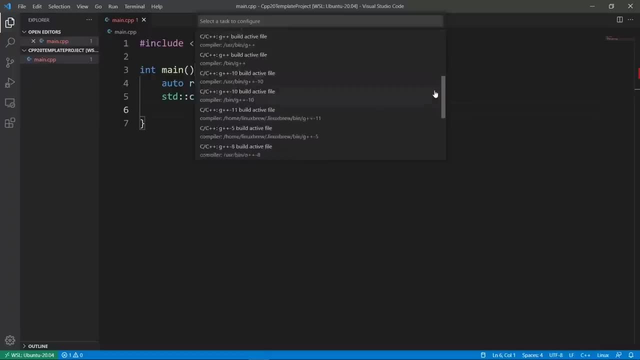 So I am going to choose the GCC compiler, which is installed through home version. This is what I am going to choose here. You see it's saying G++ 11.. But if you have access to G++ 10, you can also use that. 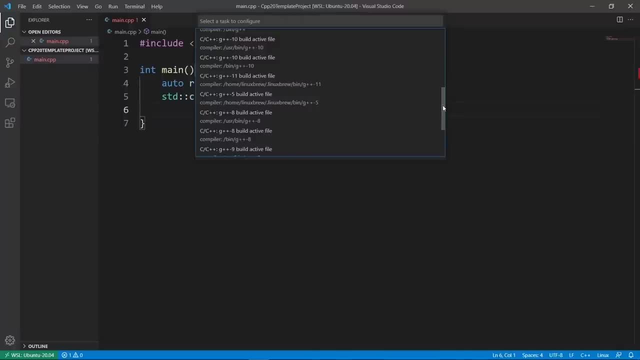 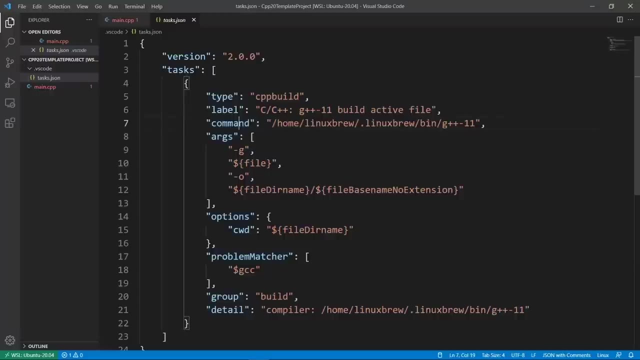 It's going to work with what we want to do in this course here mostly. So I am going to choose the best I have in terms of GCC And this is going to set up an entry in our tasksjson file to build and run this program here. 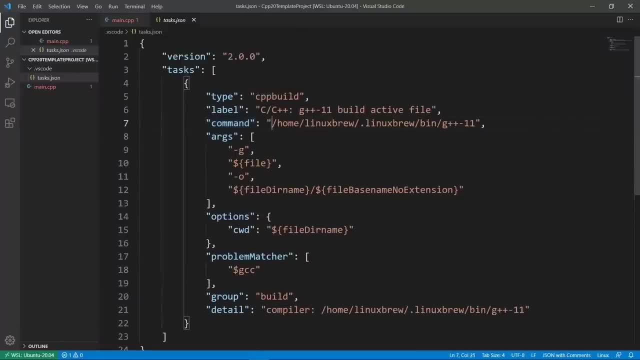 And that's what we are going to do. Okay, you see, it is using this particular compiler. And one thing we can do before we try and build this, We can change the level here to make it a little bit more descriptive. So we are going to say: build with GCC 11.2.0, if I am correct. 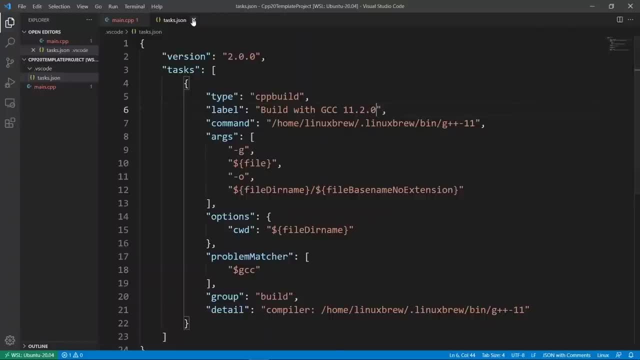 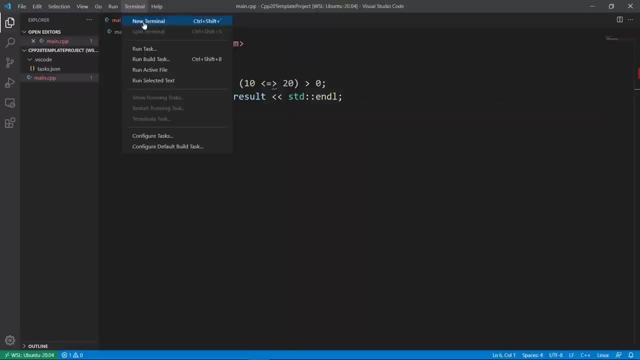 And this is all. We can save this And we can close this JSON file. And if we bring up a terminal window, we can do that by hitting terminal here and choosing new terminal. This is going to open up the current location, For example, if we do PWD in this terminal here. 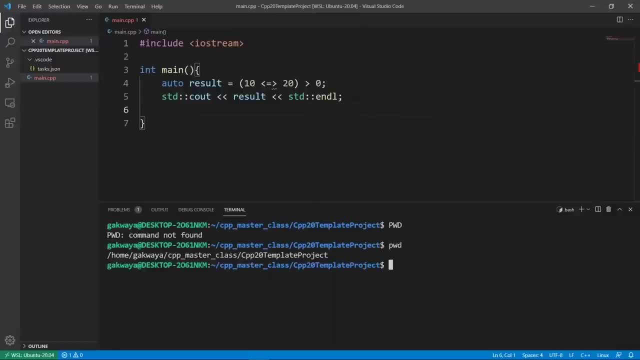 Let's use lower case. I think that's what it wants. We are going to see the location here. This is my project. So to build, I can come to terminal And I choose run task. And I am going to choose the task to compile with my GCC installation here. 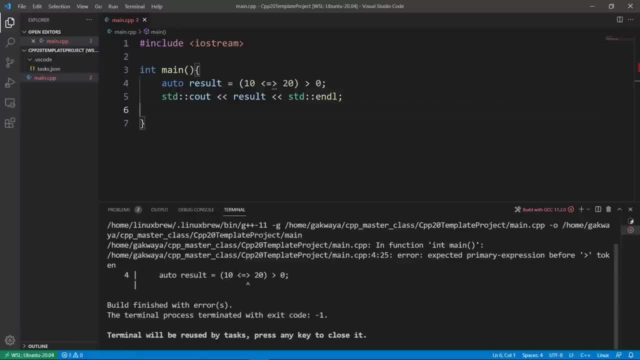 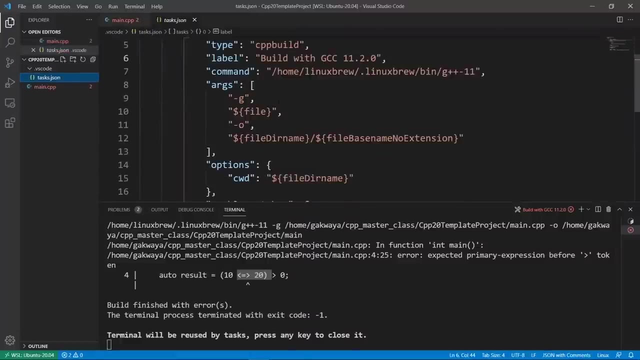 If I choose this, it is going to kick off the build process And you are going to see that the jibberish I have Is not supported because the compiler is not configured to use C++20.. So all we really need to do is go back to our command and tell it to use C++20.. 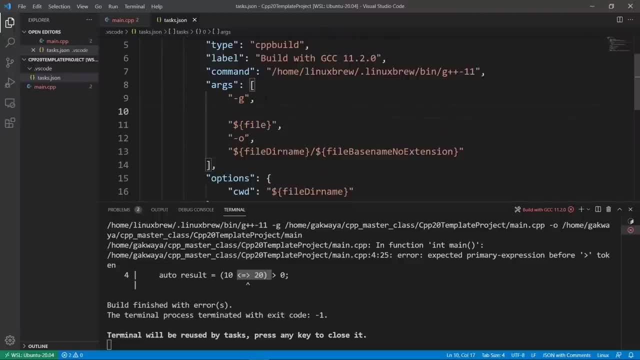 And we can do that by passing a specific instruction to the compiler to use C++20. Like we do on line 10 here. So we are going to say std equals C++20.. We are going to save this a little bit And I really wanted you to see this problem here. 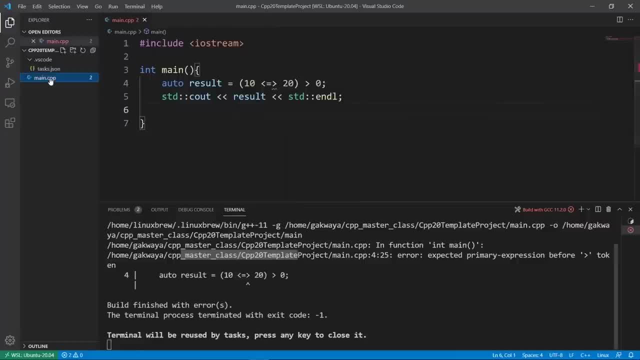 Because many people are going to forget this And we are going to try and build again, Making sure we are selecting the main CPP file here. So let's go to terminal Run task And use our compiler And wait for it to do its thing. 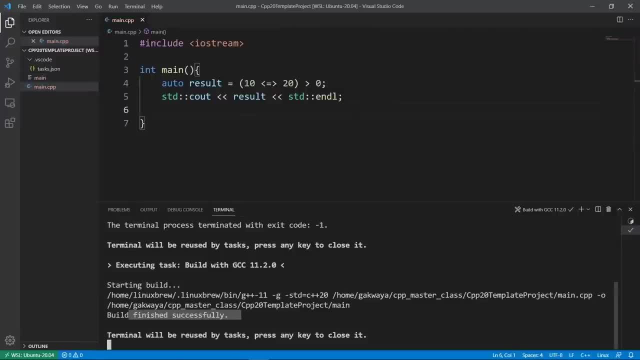 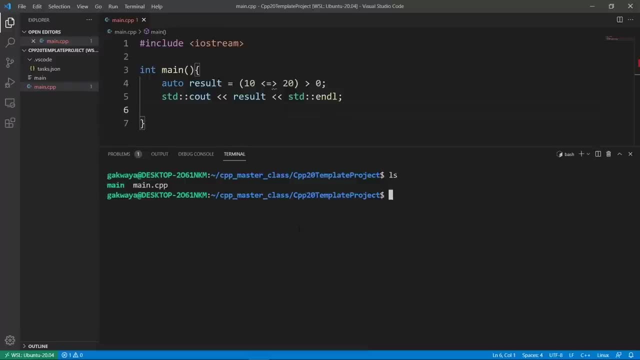 You are going to see that the build now finished successfully. And if we come back to our terminal here and do ls, We are going to see that we have a file called main And if we run it we should see a 0.. 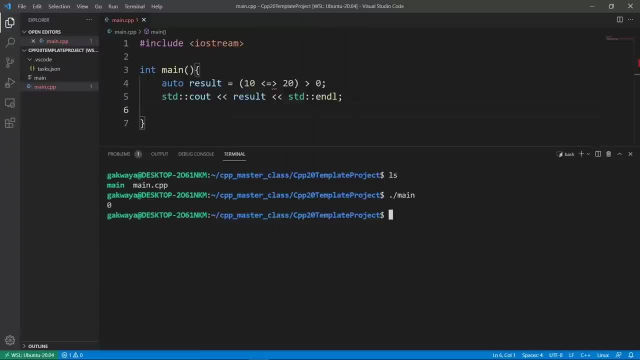 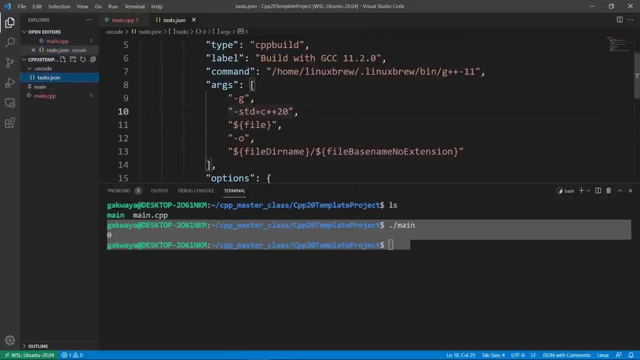 So let's say main here, And if we run it we are going to see a 0. Meaning that our program is running and working correctly. We are able to compile a C++ project on a Linux system here. Now, if you want to see how I came up with the information to use the task JSON file. 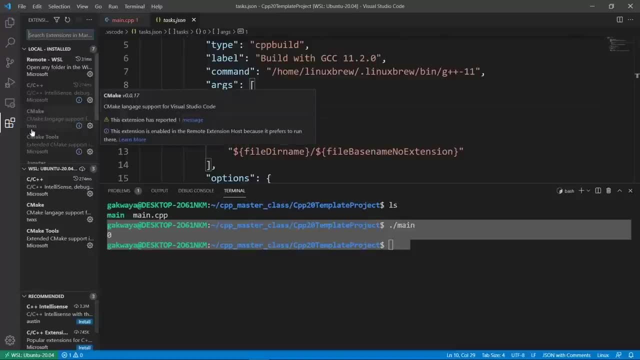 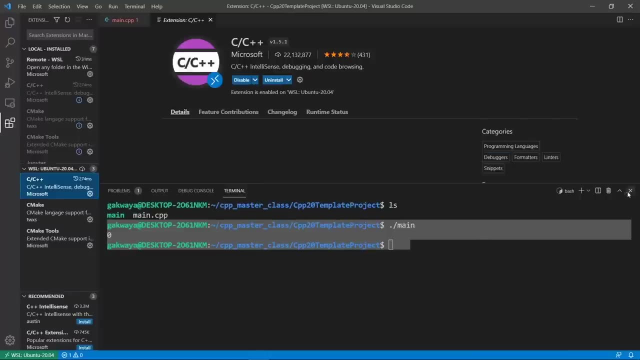 Please come back to the extensions tab here And choose the C and C++ extension. We are going to click on this And we are going to see all the instructions on how to use this guy on a Linux system here. So GCC on Linux. 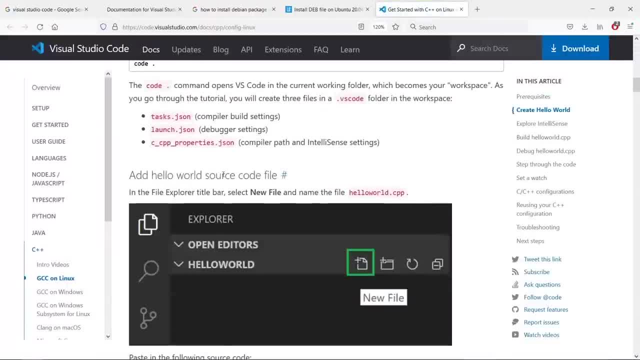 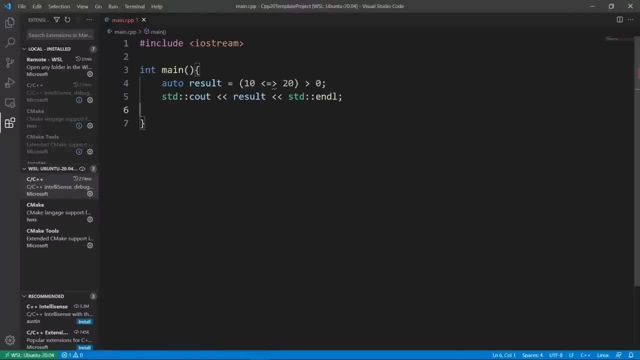 We can choose this And we are going to see all the information here Now. you can read up on all this if you want, But what I am going to do is go to Visual Studio Code And show you exactly what you need to do to get this to work. 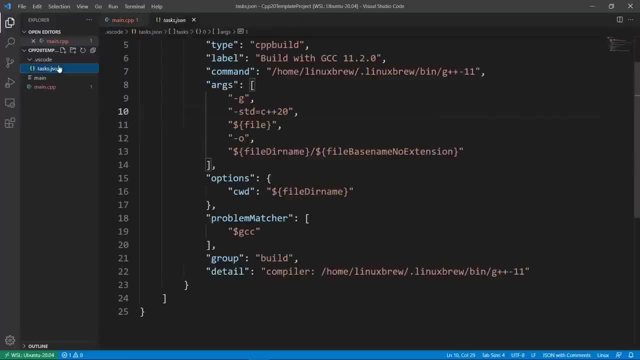 What I want to do in there is set this up to compile everything in my. What I want to do is to set What I really want to do is to. What I really want to do is to set this up So that it compiles every single C++ project. 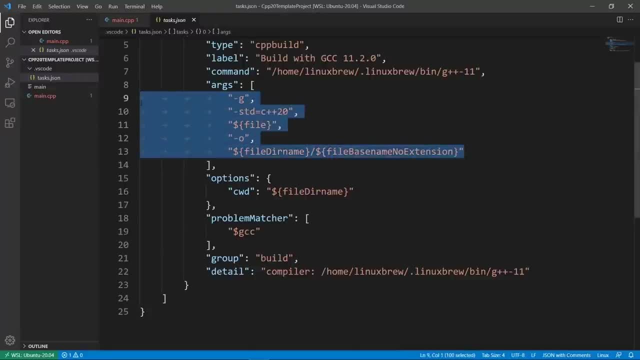 In my directory here, And I can do that by putting in a set of instructions I had prepared beforehand. So we are going to tell it to compile in C++ 20 mode. We are going to tell it to compile every single CPP file in this directory. 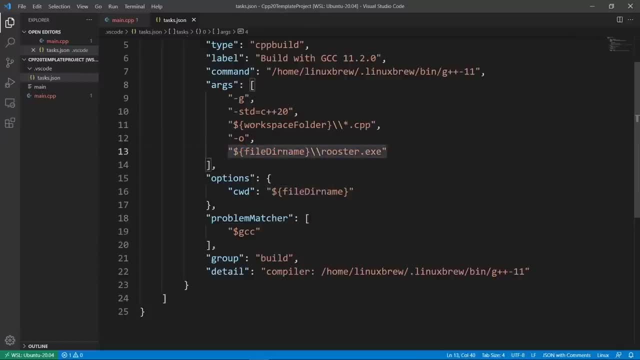 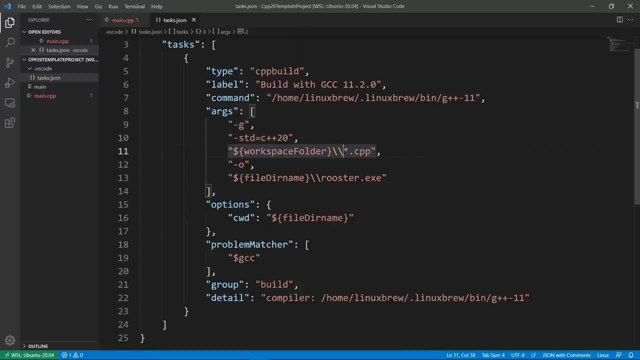 And then we are going to specify the output file name for our binary. Now this is code I used on Windows. I need to adapt it to be specific to Linux. So let's see what they say in the documentation there And we can scroll down a little bit. 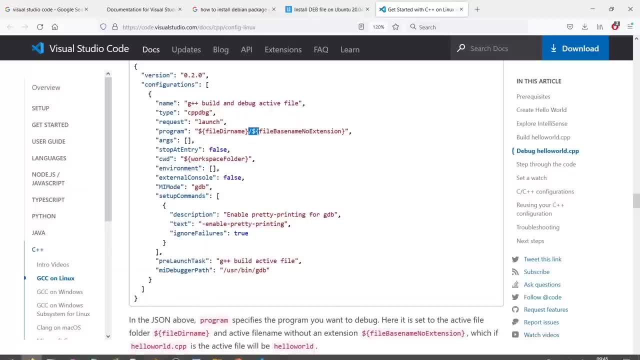 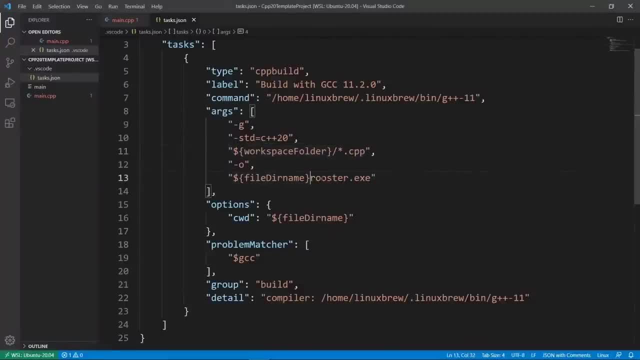 And we are going to see that they use backslashes here. So that's what we are going to use in Visual Studio Code to play it safe. So we can say this backslash and this is a backslash, And we will try and build this. 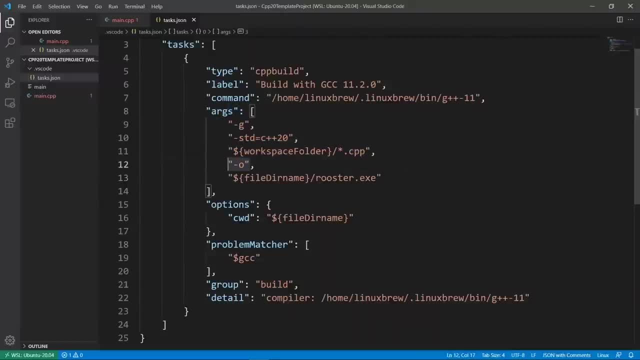 And we are going to see what happens here. This is going to build our project in C++ 20 mode. We are going to be building every single CPP file in the project And the output will be called roaster. So this is what we want to do here. 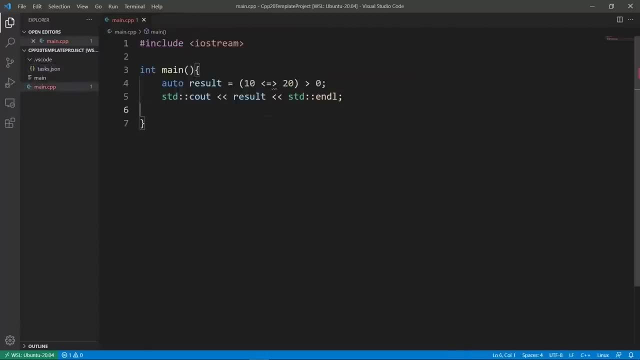 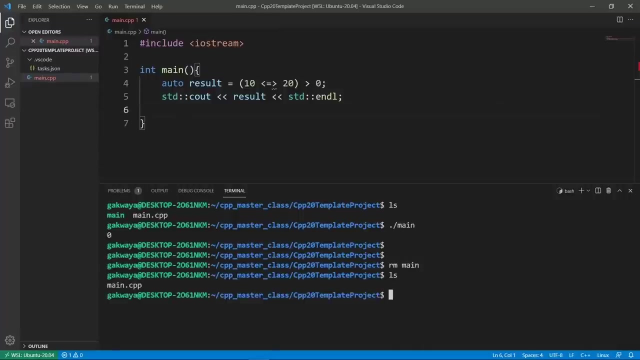 Let's save this up And I am going to close this JSON file And I will bring up my terminal by coming to view and saying terminal here And I can remove the mainexe file or the main executable I had in there. If I do ls, you see it's gone. 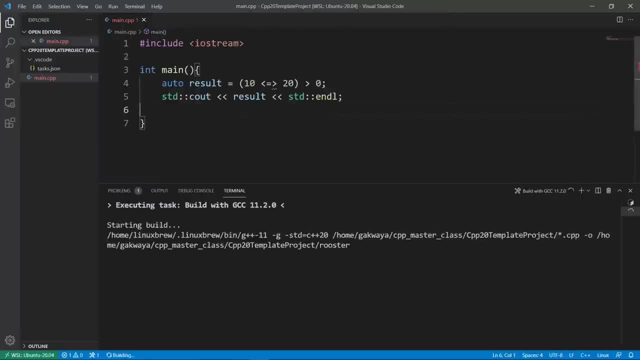 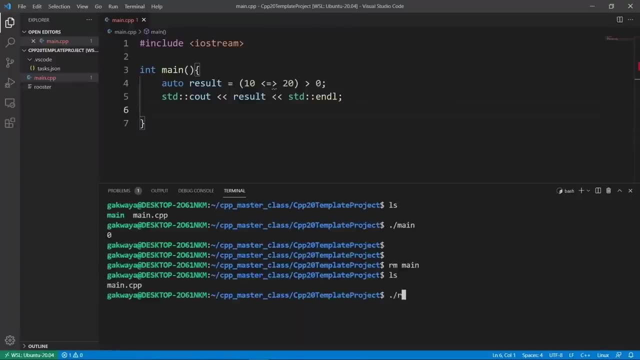 But now, if we try and compile with the GCC compiler, We are going to see what happens. You see, the build is good And we have a binary called roaster And we can run it here. If we do roaster, we are going to see it run and give us a zero. 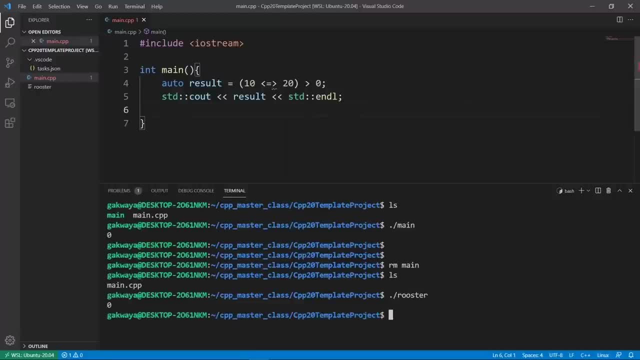 And this is really all we need to do Now. we have this working for our GCC compiler, But we want the same for our Clang compiler And we want the flexibility to be able to switch compilers by coming here and just selecting the right task. 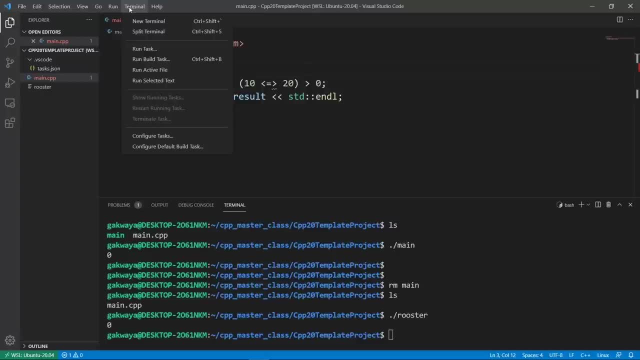 So let's do this. We are going to configure Clang, We are going to come to terminal, We want to configure a task And we are going to choose the best we have in terms of Clang. That happens to be Clang++12 here. 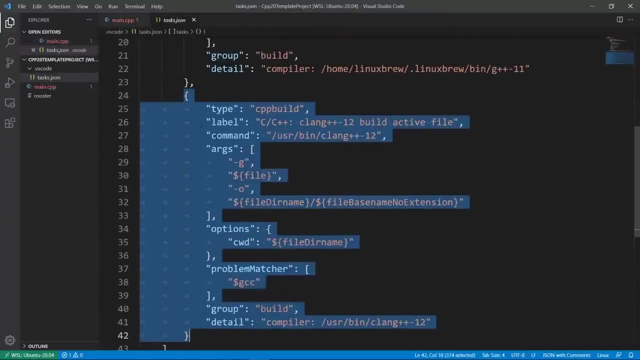 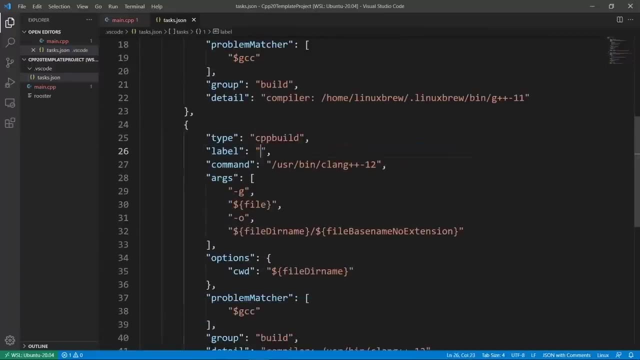 So we are going to choose this And this is going to add an entry in our tasksjson file. We are going to change this to say that we want to build with Clang. Let's do that. We are going to say: build with Clang. 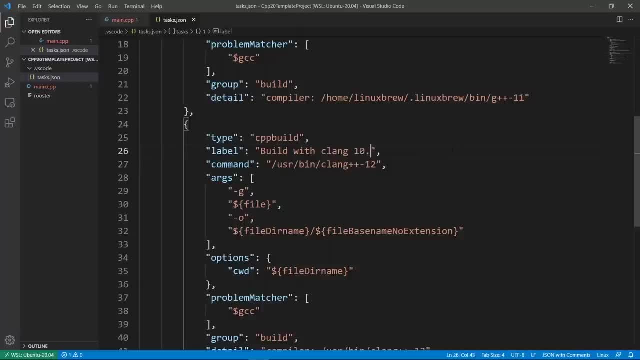 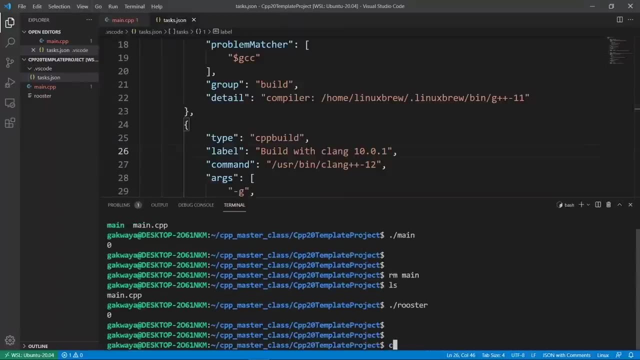 I think we have 12.0.1, if I remember correctly. But we can ask our terminal here. Let's go to terminal And we are going to say Clang++12.. That's the version And we are going to ask it. 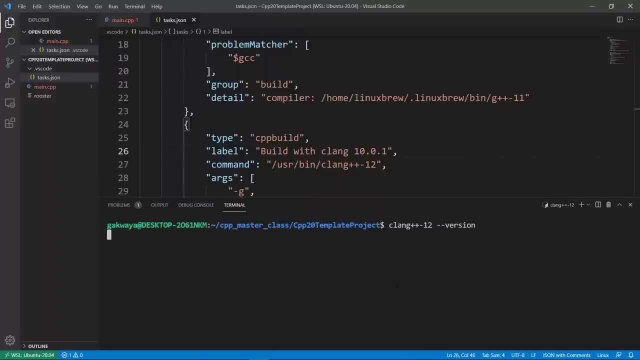 What's your version? It's going to tell us in detail And if we wait, we are going to see this speed out on the terminal here, And this happens to be Clang version 12.0.0.. So that's what we are going to say in our file here. 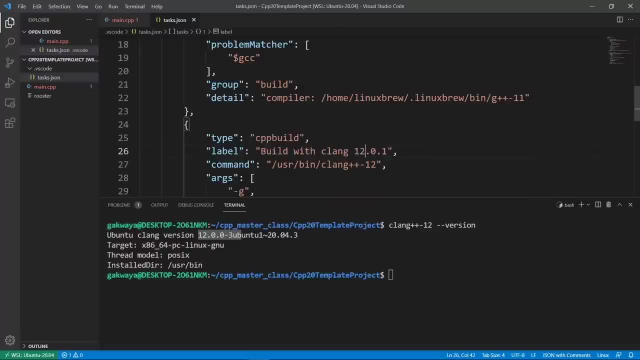 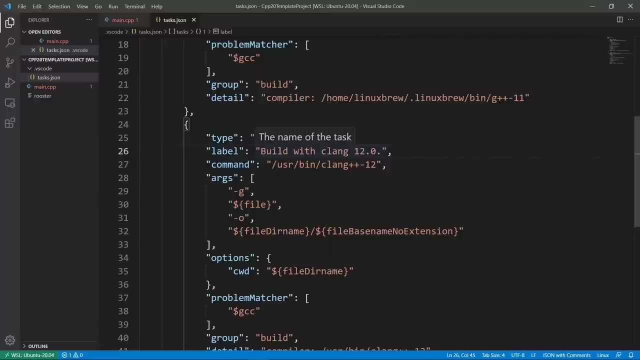 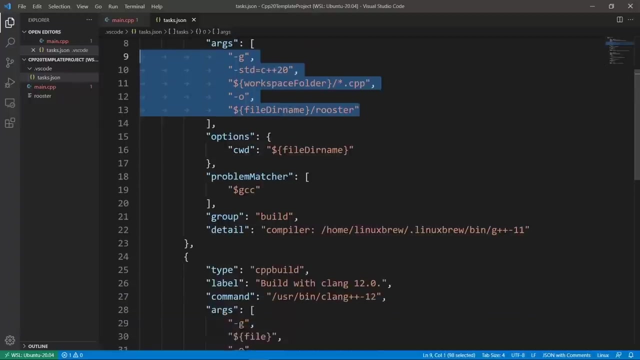 Build with Clang 12.0.0.. To be super clear on this, And this is really all. All we need to do is put in the instructions to build in C++20 mode, Exactly what we did for GCC here. So I am going to copy this and put that in my arguments here. 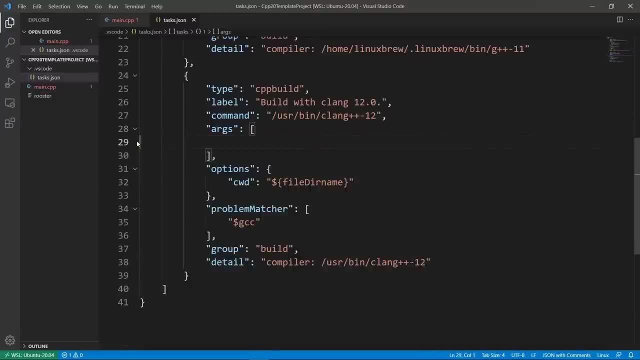 I am going to take out whatever I had in there. I am going to put in my new things And let's see if this compiler works. now We are going to save our tasksjson file And come back to the CPP file. We are going to bring up our terminal window. 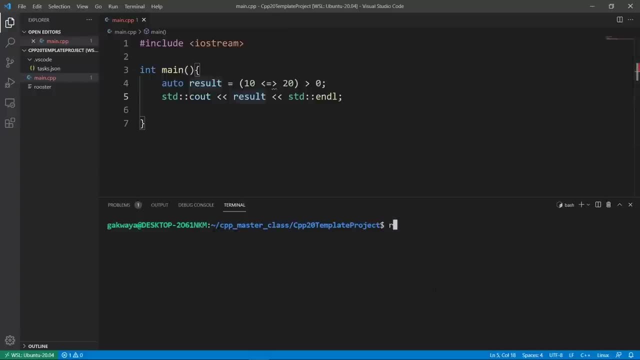 And we are going to clear And remove rooster Because we want to build a new one with our Clang compiler And we will come to terminal Run task. Now we are going to choose to build with Clang 12.0.. 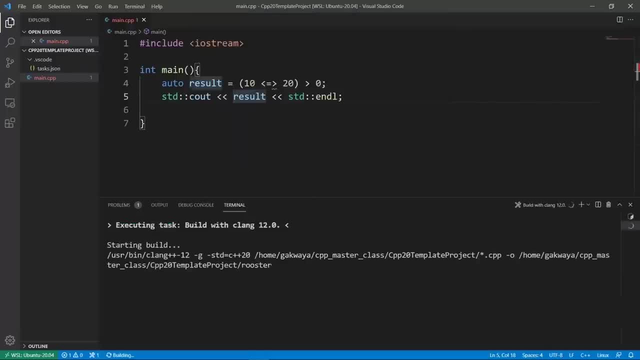 We are going to fix this in a minute, But if we do this, we are going to see that our build process is going to start. It's going to be building with our Clang compiler. It's going to be using C++20.. 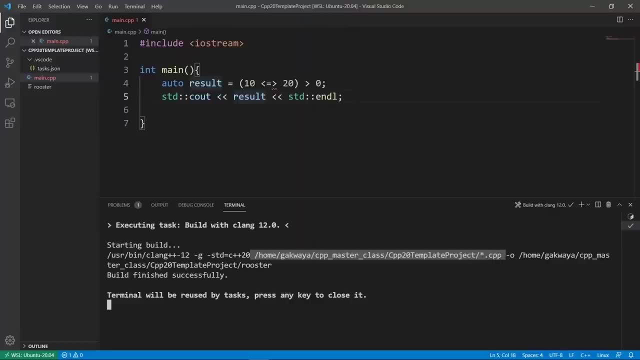 It's going to be building every single CPP file in this location here, And the output of this And the output of the build will be a binary called rooster that we have right here. So the build is good. If we do ls, we are going to find rooster. 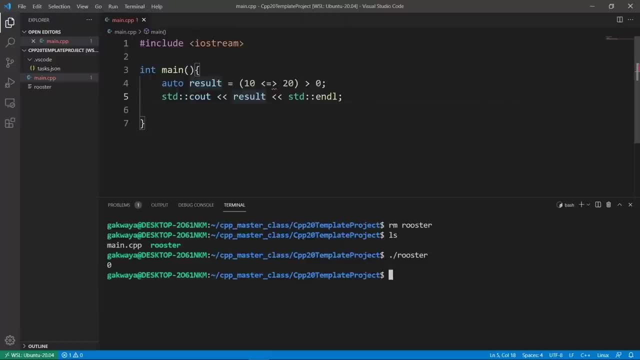 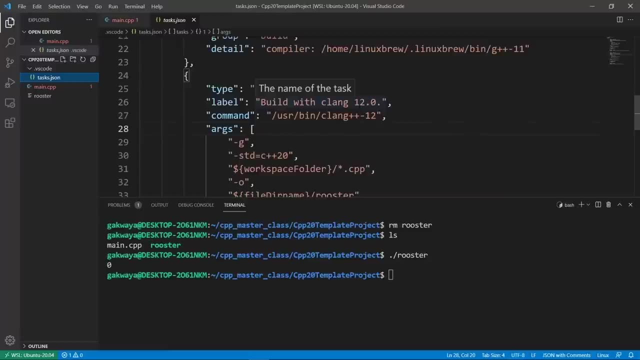 And if we run it, it's going to say 0.. Exactly as we expect here, And we have Visual Studio Code properly configured to use our two compilers, The Clang compiler and the GCC compiler. Let's come back to our configuration and change this to say 12.0.0.. 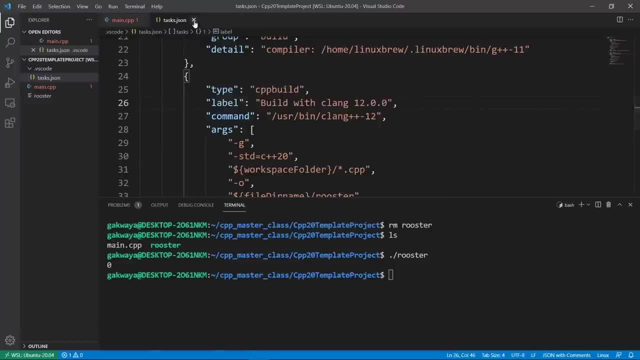 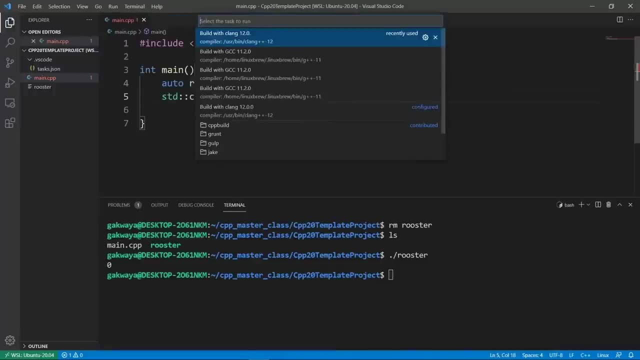 To be super clear on the version we have. We can close our JSON file here And come and try to build again. If we do terminal and run task, we will have our compiler here. Ignore all these things. I think Visual Studio Code is going to give you duplicates. 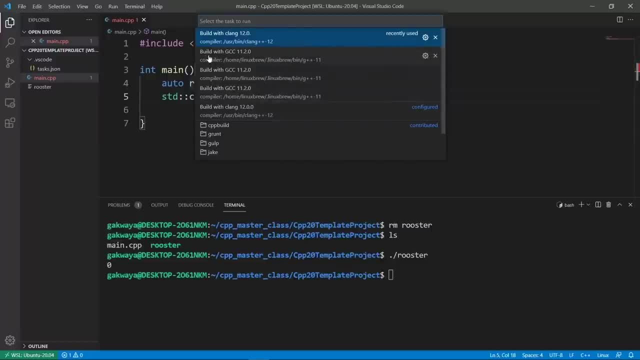 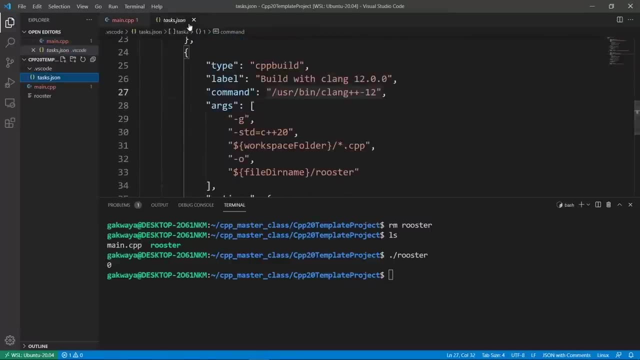 But you can choose the version that says what you want And it is going to work. So we are going to choose GCC. Oh, we are saying GCC, But we want Clang here. So let's say that we want to build with Clang. 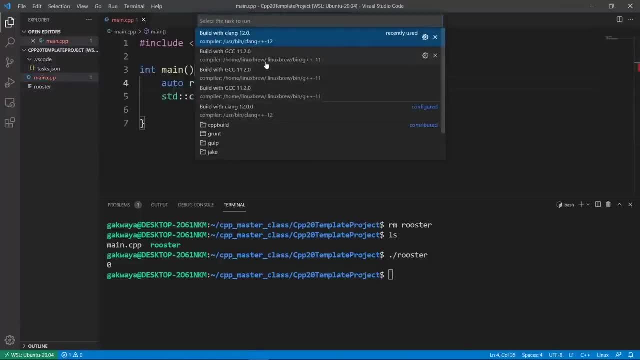 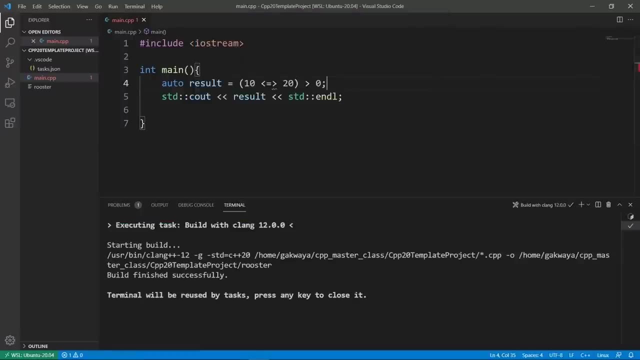 We are going to go to terminal And run task And we want Clang 12.0.0.. This is right here, So we are going to select it And it is going to work successfully And we will have our binary here. 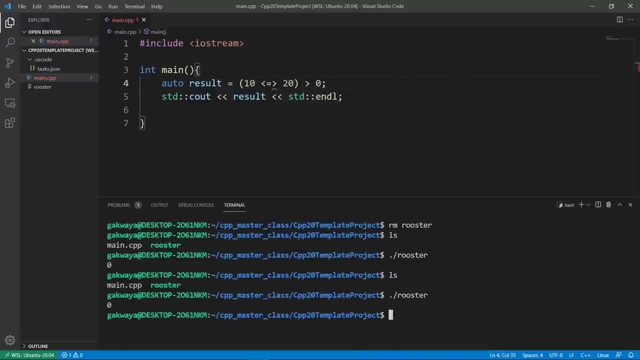 If we run it, it is going to say 0. And this is really what we need to do here. So this is really all I had to share in this lecture: Showing you how you can configure Visual Studio Code to compile using the compilers that we have installed. 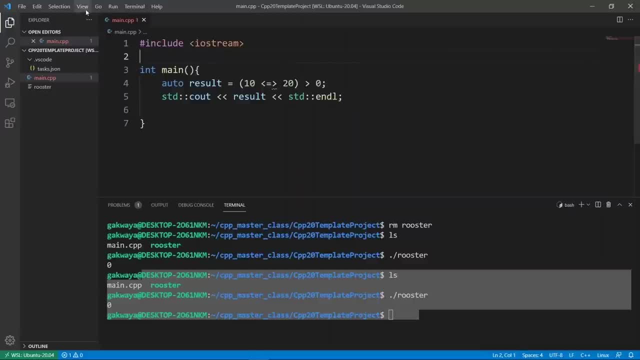 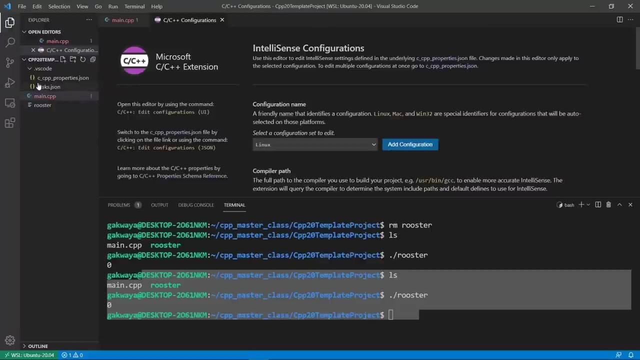 Another thing you can do to make your experience better Is come back to view And select command palette here And you can do C and C++ And edit the configurations through a user interface. And if we do this, you are going to see that this is going to create a CPP properties JSON file. 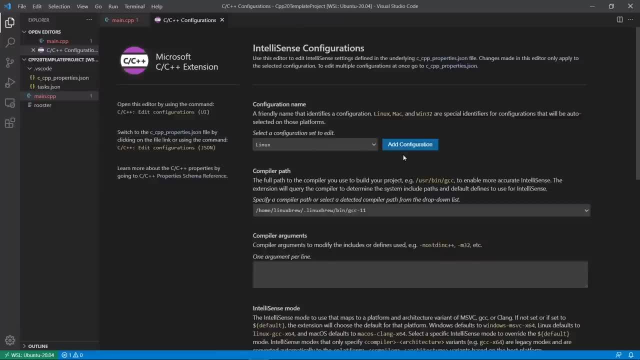 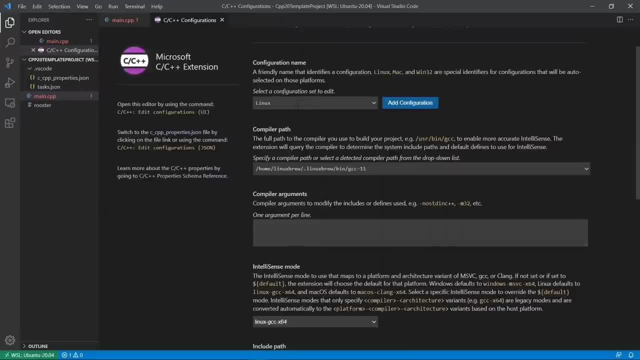 So this is where we can configure what kind of Intellisense, What kind of compiler is going to be used. We can do all these things here, So we are going to leave it to the default. It is on our Linux system. 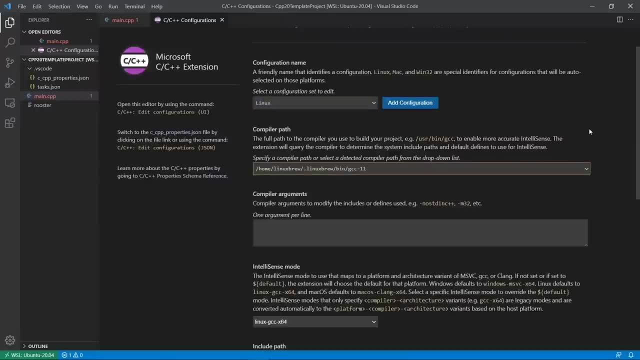 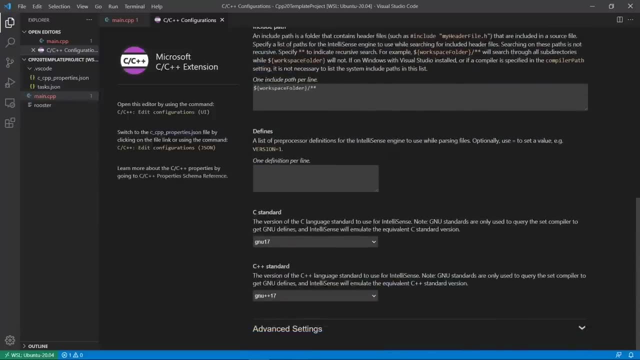 We are going to be using GCC 11. Which is the best we have in terms of GCC. But one thing you should note in this course here Is the C++ standard we want to use, So we want to use C++ 20.. 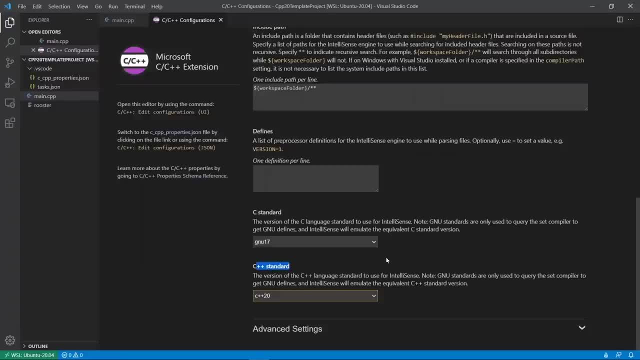 And we want Visual Studio Code to give us Intellisense Or format our main CPP file based on the C++ 20 standard here. That is what we can achieve with this. So once you have this in, You can come and close this. 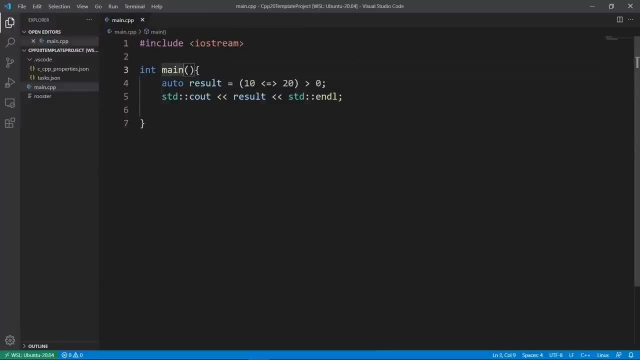 And if we go back to the main CPP file, You see now that this is no longer flagged as a problem with squiggly lines. Visual Studio Code is properly understanding what is happening here, And this is something you can do to make your experience a little bit better. 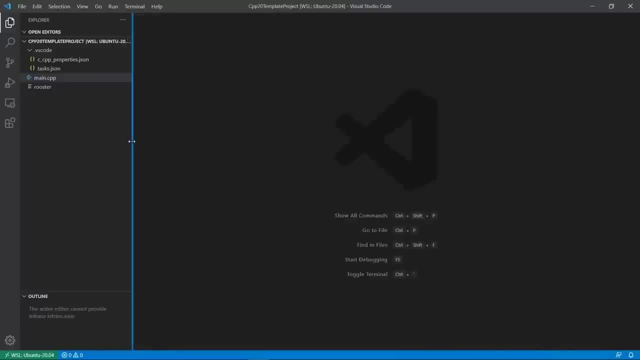 Okay, now that we have this project set up and ready on Linux, We are going to be reusing this as a template project Every time we start something new on Linux. So every time we want to create a new project, We will grab this entire folder. 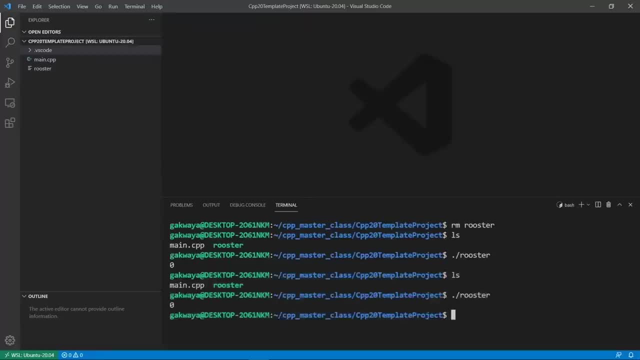 So, for example, we will come to our terminal here And go up a little bit, So cd, and go up one level, And if we do ls, we are going to have our C++ 20 template project. We will copy it and rename it to start a new project. 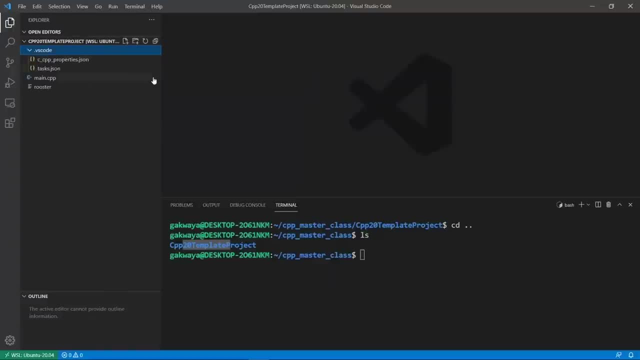 And that is going to give us all the configuration that we did. We don't need to reconfigure the compilers or whatever. It is going to work right out of the box. And that is really what we did here. We set up a template project. 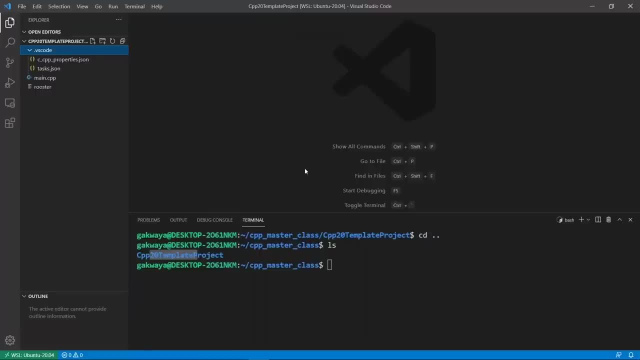 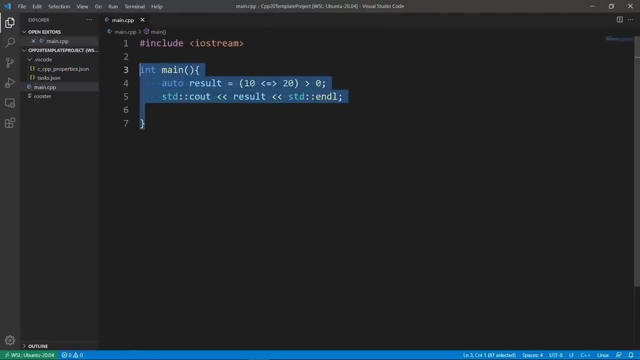 That we will be reusing all over again in the course as we progress, Learning about C++ 20.. I am going to stop here in this lecture. In the next one I am going to show you how you can set up a development environment. 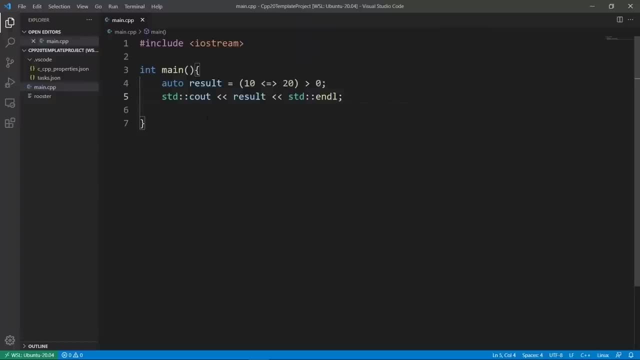 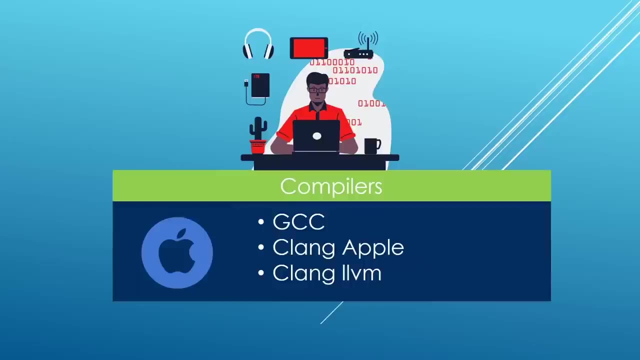 On the Mac OS system. Go ahead and finish up here And meet me there. In this video, I am going to show you how to install C++ compiler on your Mac OS system And we have a bunch of options. On the Mac, we can install the GCC compiler. 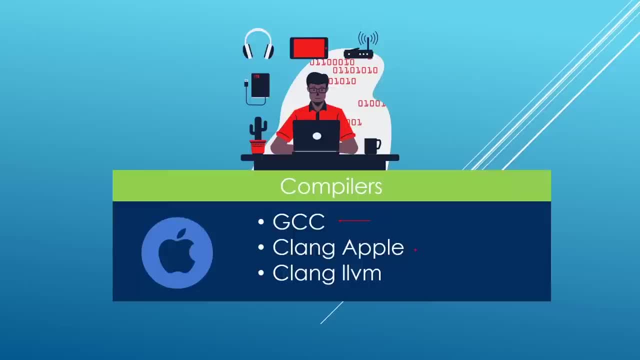 We can install the Clang version of the Apple company, Or we can install the Clang LLVM version. All these are options And I will show you how to install these. I don't have access to a Mac device, So I won't really be able to install Xcode and show you. 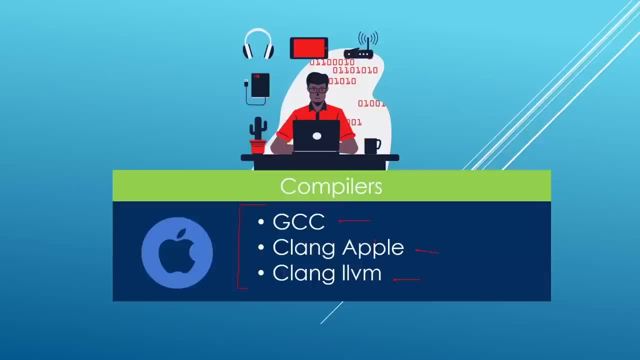 But I think you can manage. if you are using a Mac system, It is nothing complicated. You just have to go to the Apple store And click on Xcode And it is going to install For GCC and Clang LLVM. I will show you how to do this using the Homebrew package manager. 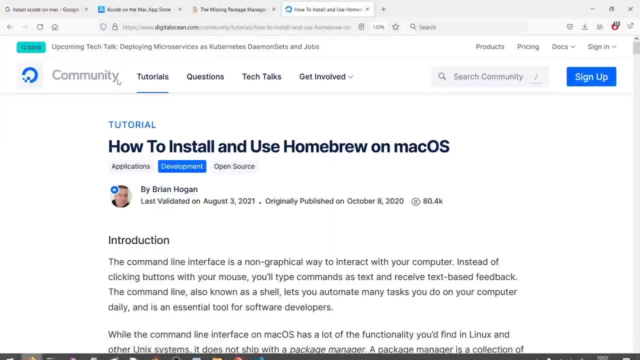 Which is also going to make this super easy. Okay, so let's head over to our browser, And we have a good link here from DigitalOcean On how to install and use Homebrew on a Mac OS system. This is a really validated link. 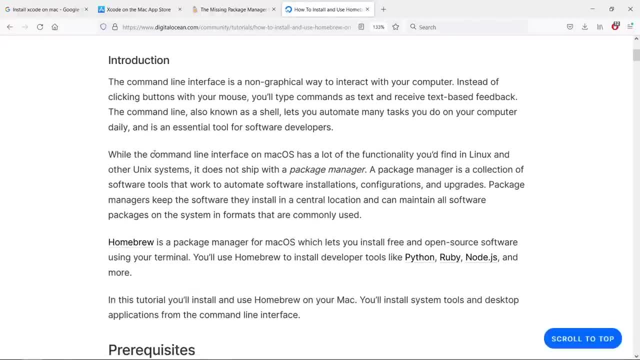 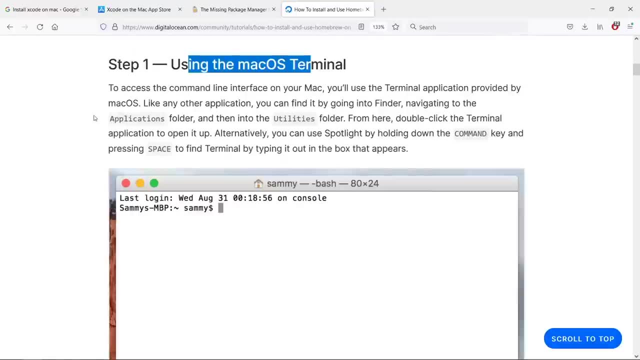 You can see that right here And you can read up on this. if you are using a Mac system, I am going to share the link here In the resources section of the course And to use this We will go through the Mac OS terminal. 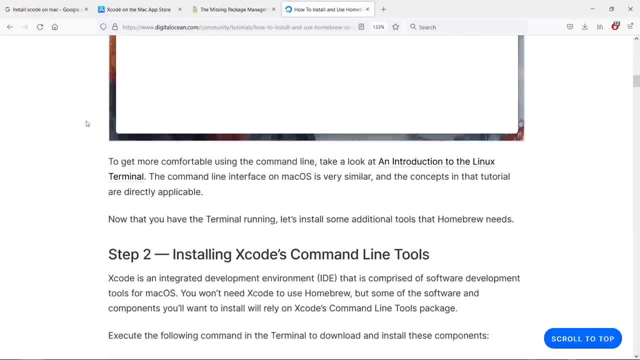 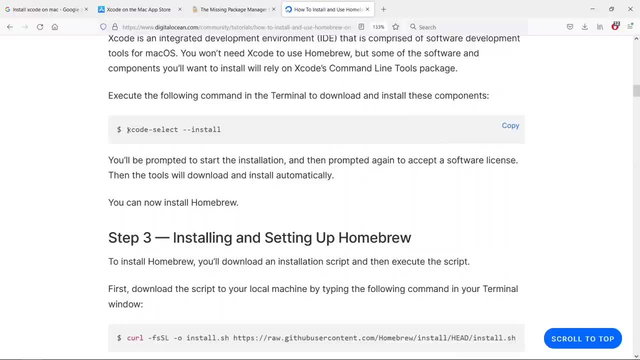 And it is nothing complicated. You can search for it and open it up, And after you do this You will have to install the tools needed to build things on the Mac OS system, And that is going to install Xcode here, So grab the command here. 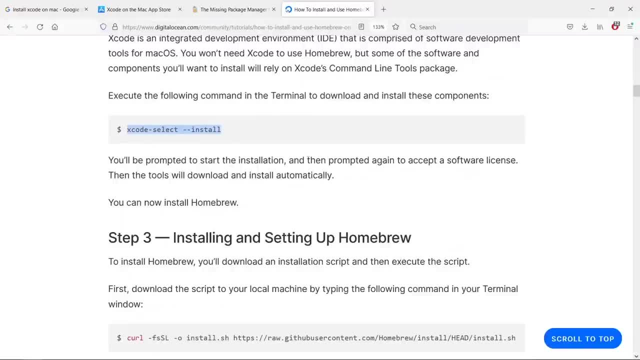 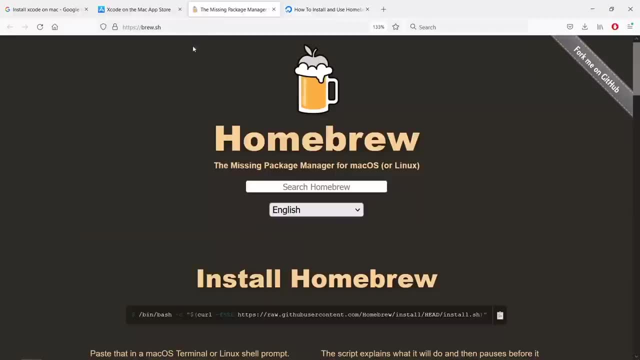 And run it in your terminal And this is going to install everything you need And after you have this installed, You are going to install Homebrew. I do recommend coming up to the website here For Homebrew And clicking on this copy icon here. 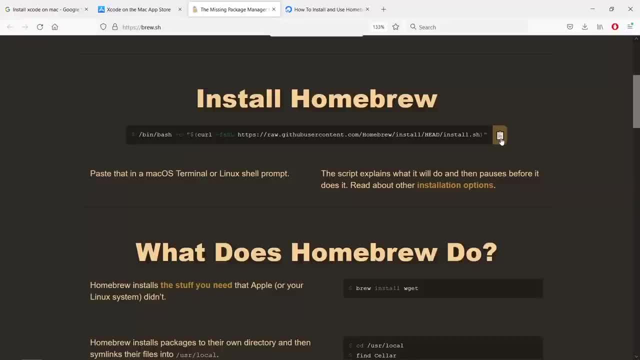 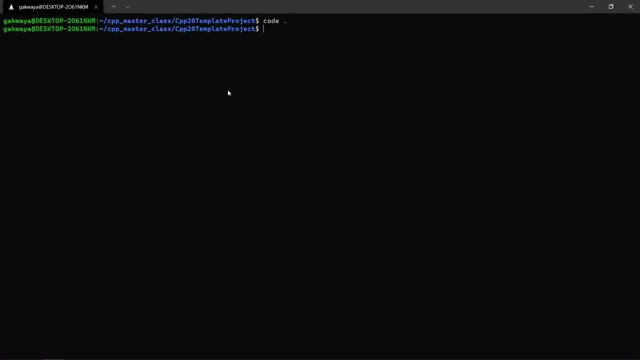 This is going to copy the entire thing And you can copy this And once you copy it It is going to give us a green tick here And you can go in the terminal on your Mac OS system. I am using a Linux terminal here. 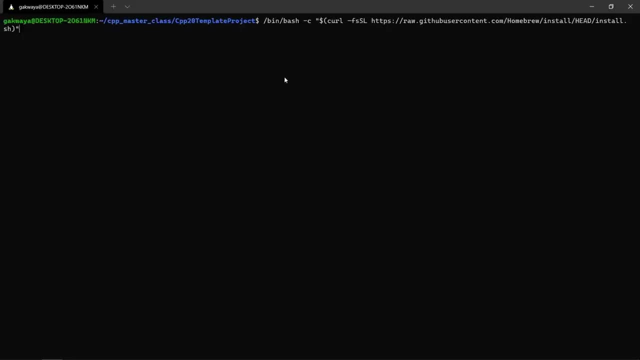 And then you are going to paste this command in here And hit enter. Once you do that, It will be prompted to put in the password. It is going to tell you that it needs to install Homebrew, And you are basically going to wait for this to finish. 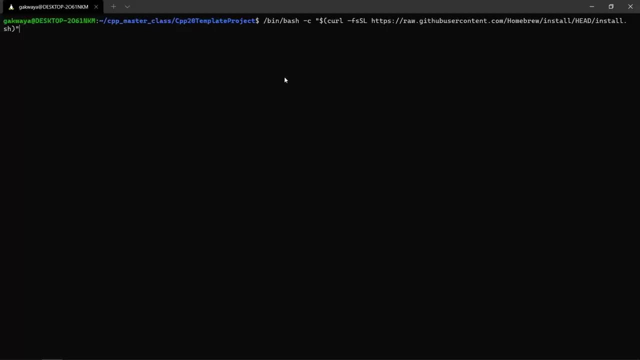 I have to warn you This is going to take some time. Even if you have a good internet connection, This is going to take some time, So be patient here. When it is done, It is going to tell you that it is finished. 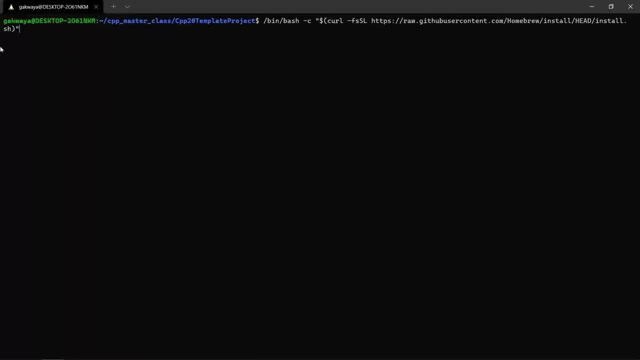 And you will be ready to install the GCC compiler And the Clang LLVM compiler Through your Homebrew installation here. I am not going to click on this, Because I already have this installed On my Linux system here. Let's go back to the link. 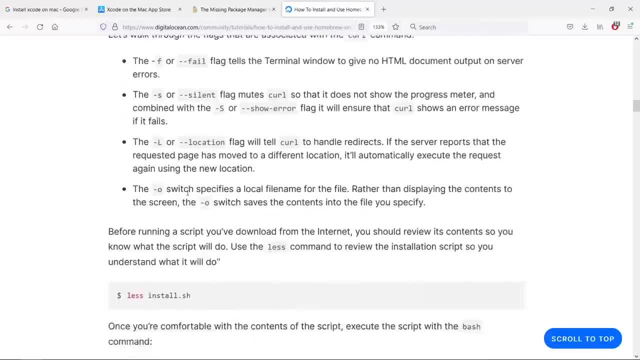 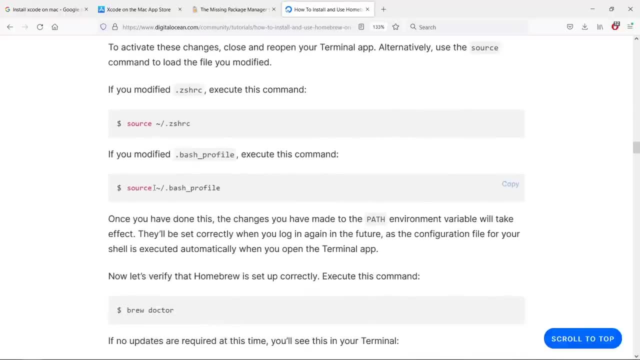 And see what they say next. So after you paste that in, It is going to install And after that You will see that Homebrew is going to be installed on your system And you can use Homebrew To start installing and upgrading packages. 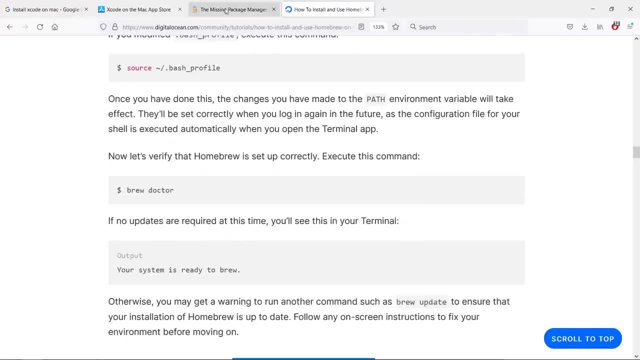 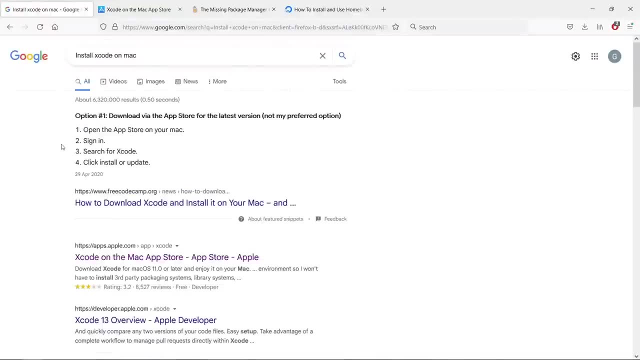 You can really read up on this. But what I want you to see Is that you can use Homebrew To install the GCC compiler And the Clang LLVM compiler. So if we come to the search here And say GCC, Homebrew- 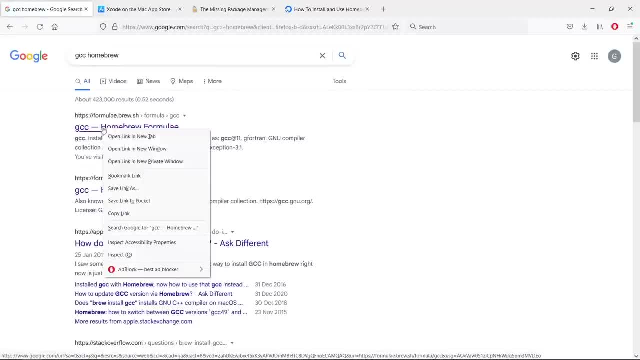 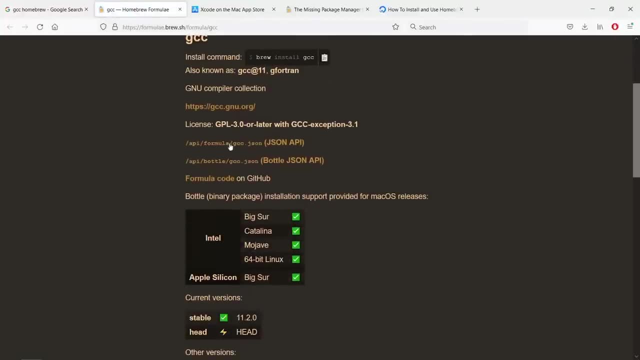 We are going to find instructions On how to install this. So all you need to do really Is to say brew, install GCC. This is going to install the latest version Of GCC on your Mac. If we come here And say LLVM or Clang. 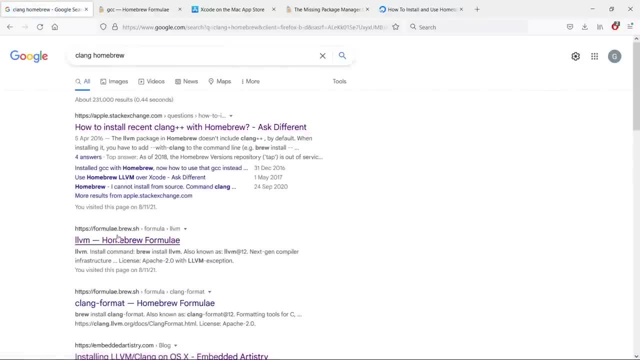 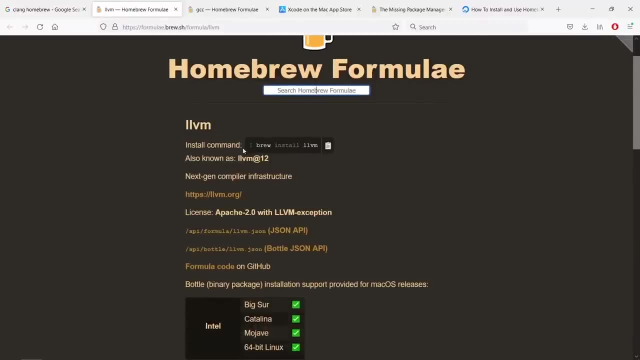 Let's say Clang, And we can find that right here- LLVM, And it is going to give us instructions On how to install this, And all you have to do Is brew, install LLVM, And this is going to install these two compilers. 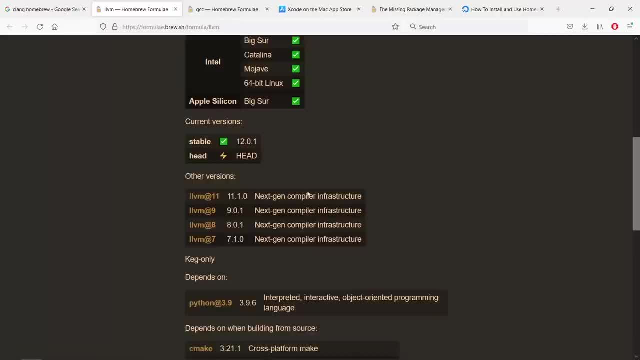 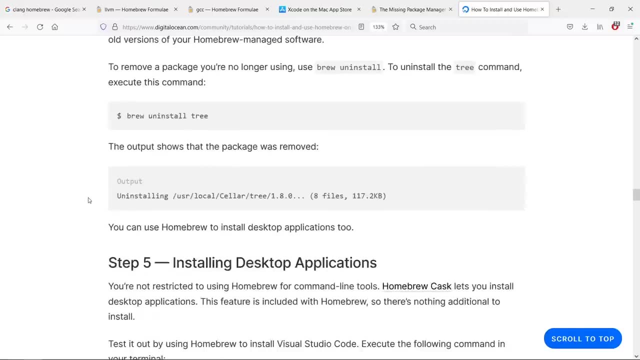 On your Mac system. So once you do that, You will have them stored somewhere. Let's go to the install link And we are going to see that Homebrew is basically going to be installed And thanks, in your user local Directory on a Mac device. 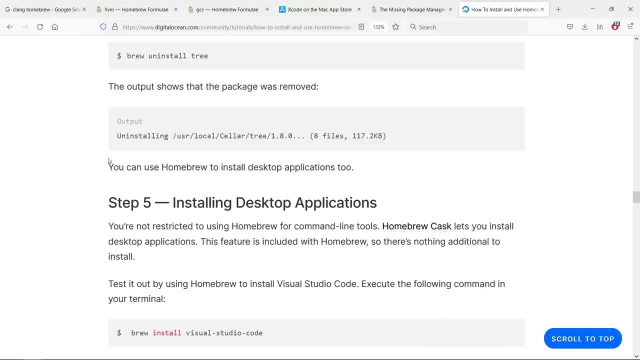 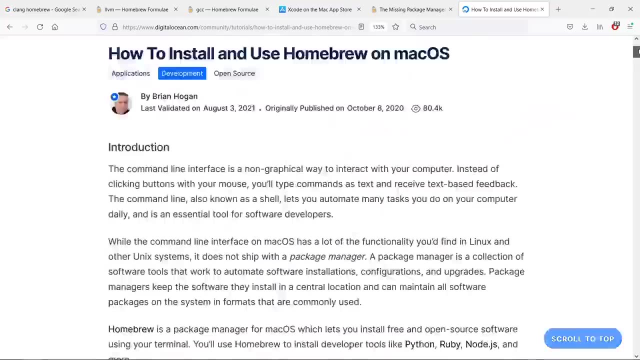 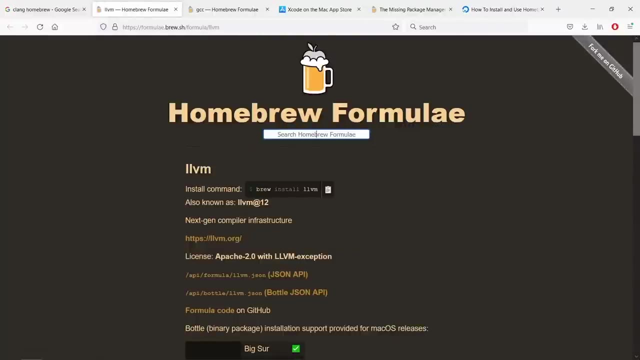 Please tell me if this is true For your case And if you have a problem, Please do that And fix that up. So if you are on a Mac, I would really recommend going through this To install homebrew Once you have that installed. 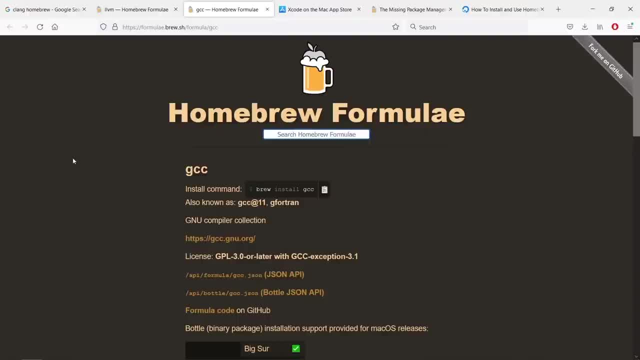 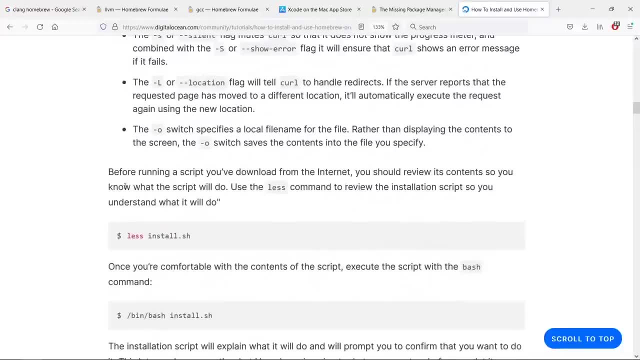 You will go through that To install both of the LLVM compiler And the GCC compiler And that is going to give you the latest versions For these compilers. To find out if they will install, You can go in your user local directory. 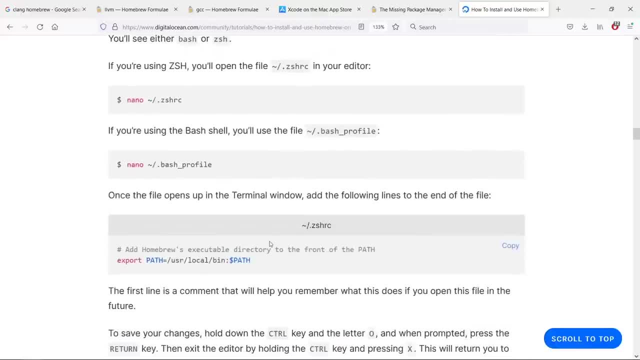 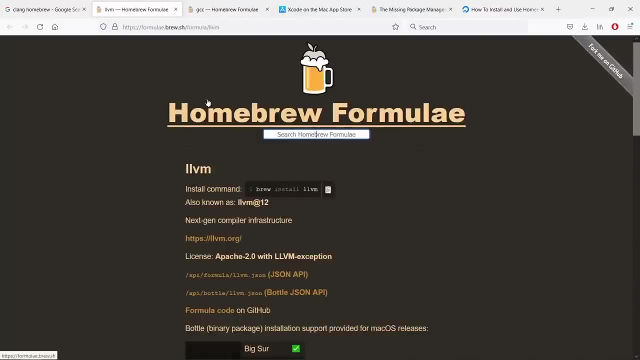 And you can hunt for these compilers And start using them To build your C++ applications. So by now I am going to consider That you have both GCC and Clang installed On your Mac system, The next logical thing to do. 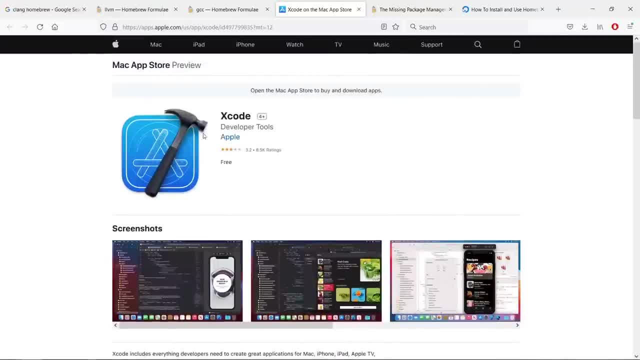 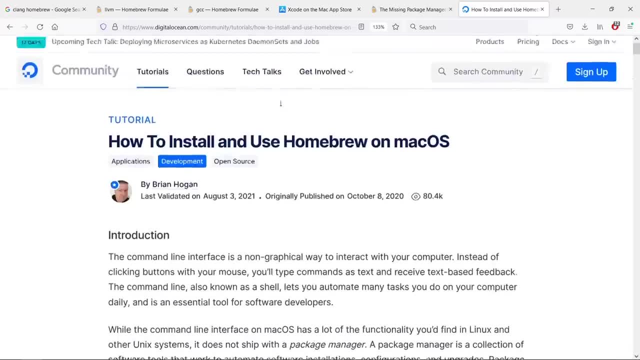 Is to want the Apple version of Clang, And I think that is going to come As part of Xcode here And it is going to come As a result of running The command that we did before. I think it was this little command here. 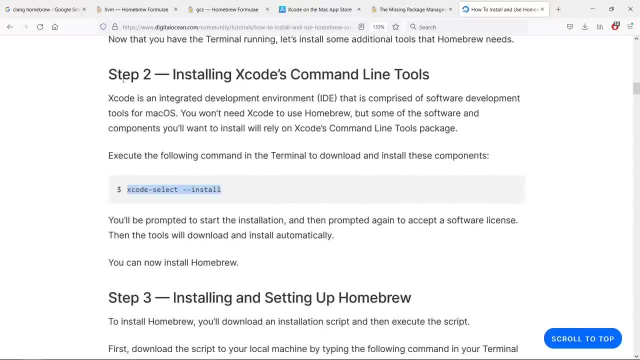 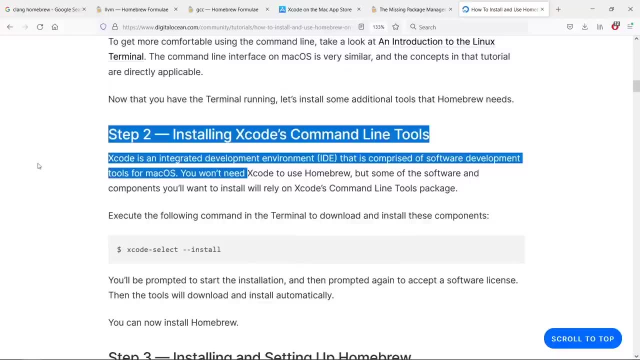 Which is going to install everything you need, From the Xcode To the Mac OS IDE. So this is all I had to share in this lecture. Again, I apologize. I don't have access to a Mac device, But if you have a problem you can tell me. 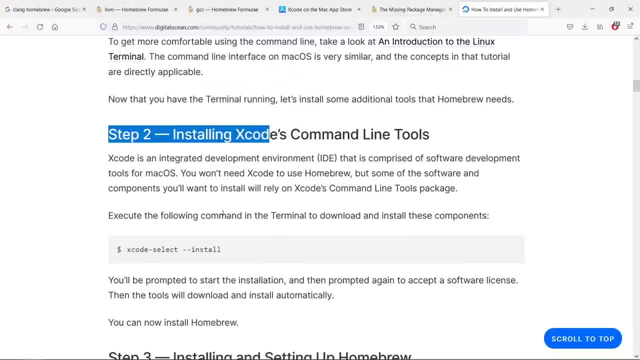 And I will try to help you out And get this sorted out. We are going to stop here in this lecture. In the next one we are going to see How we can install Xcode on your Mac device. Go ahead and finish up here. 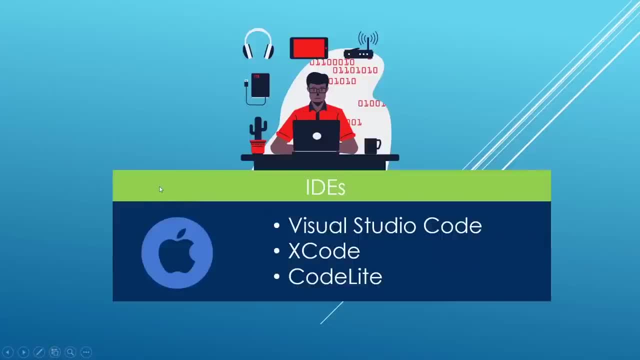 And meet me there. In this video, I am going to show you How to install the Visual Studio Code editor On your Mac OS system. Please know that you can also use Other IDEs like Xcode or CodeLite. Do C++ development. 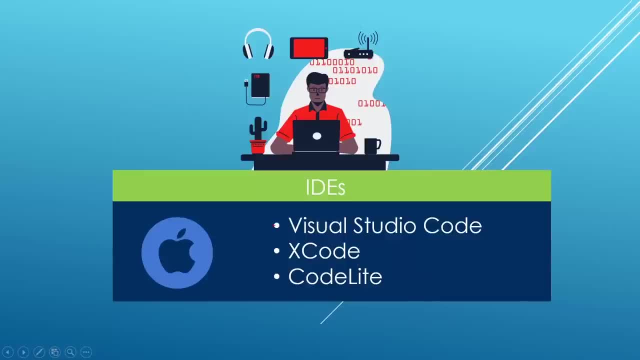 But Visual Studio Code is going to be Our main editor In this course here And I would recommend to install it So that we are doing consistent things. That is going to reduce chances For you to get confused. So we are going to head over to the website. 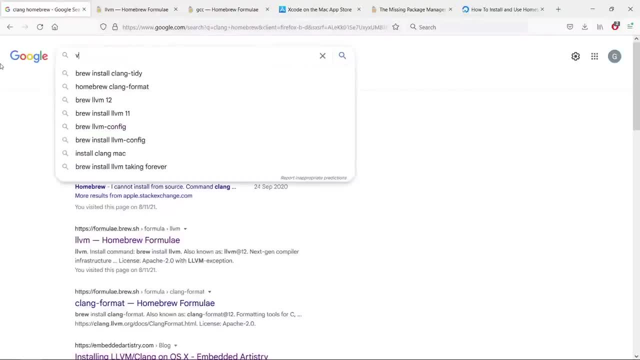 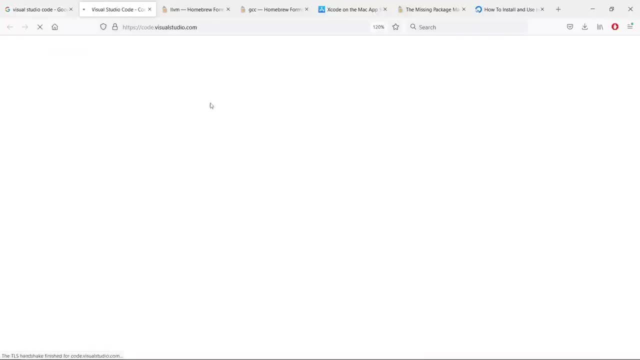 For Visual Studio Code And to get there we can just type Visual Studio Code in here In our search engine And we will have a link here That we can use to download our things. So we are going to go down And find download links. 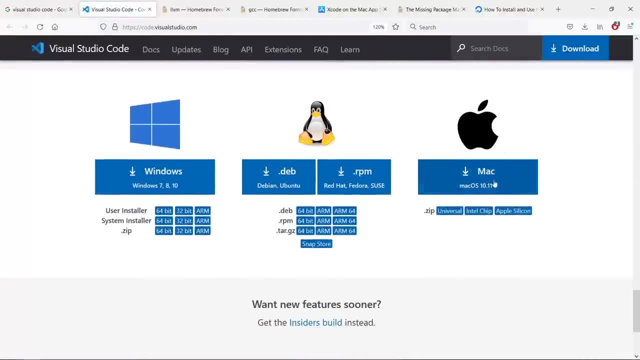 For Windows, Linux and Mac. Please use the Mac download button here And you are going to download The binary and install it. I think it is going to be in The download folder by default, So all you have to do is drag that up. 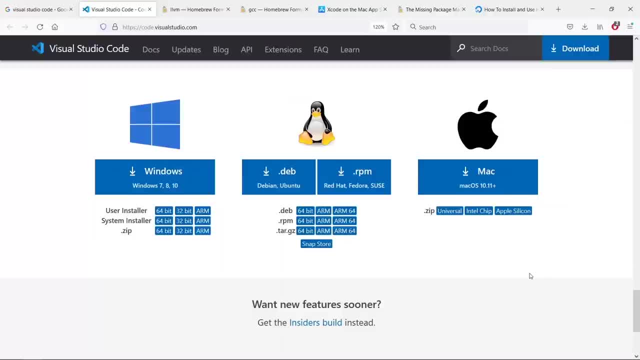 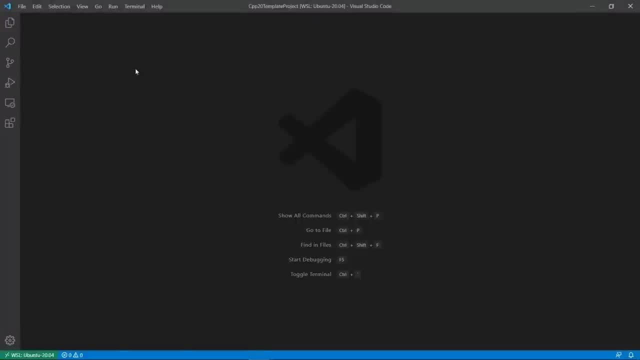 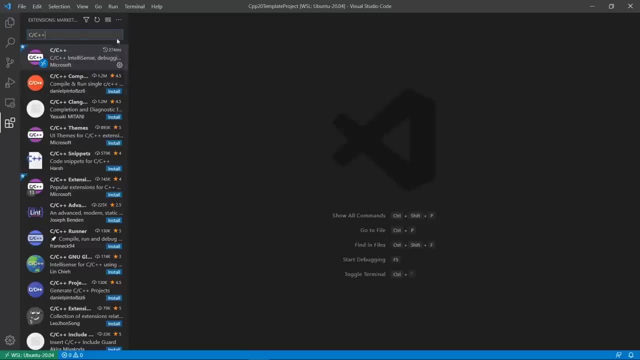 In your installation directory So that it becomes A runnable application. After you do that, you are going to run it And you will have A user interface like this With Visual Studio Code opened up. Once you have that up, You will need to install the C++ extension. 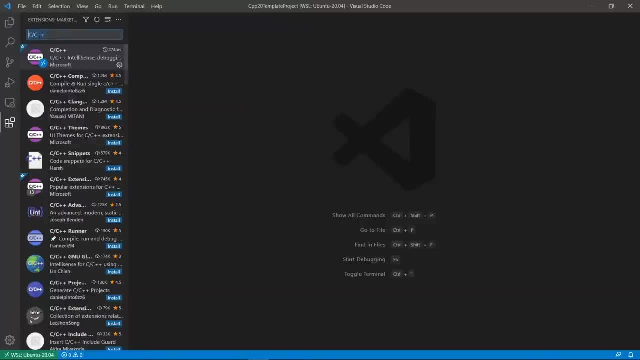 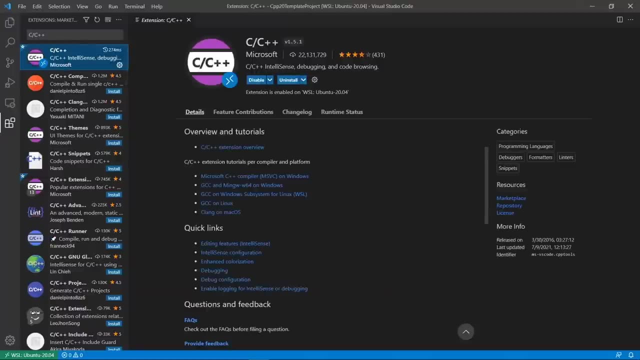 And what you need to do is come to The extensions tab here And type C and C++ in here And you are going to have an entry for Microsoft. Click on that And install this extension on your system And your Visual Studio Code instance. 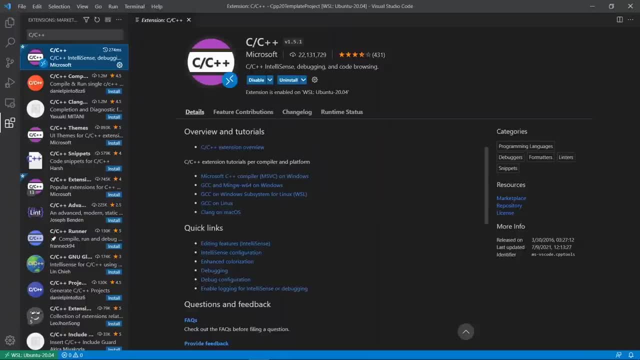 Is going to be ready to handle Some C++ development, And this is really all That I had to share in this lecture, Showing you how you can get this installed. Again, I apologize, I don't have access to a Mac device, So I used my Linux box. 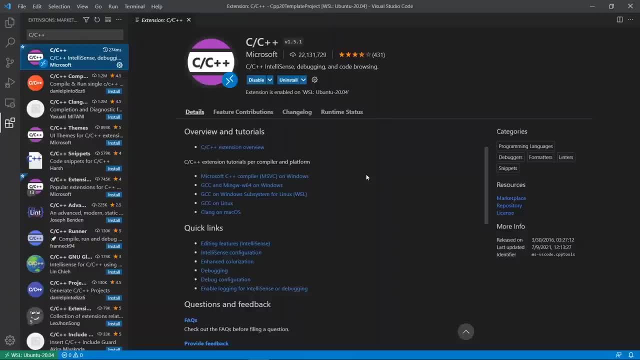 Running inside Windows subsystem for Linux to show you this. But this is good enough, I think. If you have a problem, you can tell me And I will do the best I can to help you out. For now we are going to stop here. 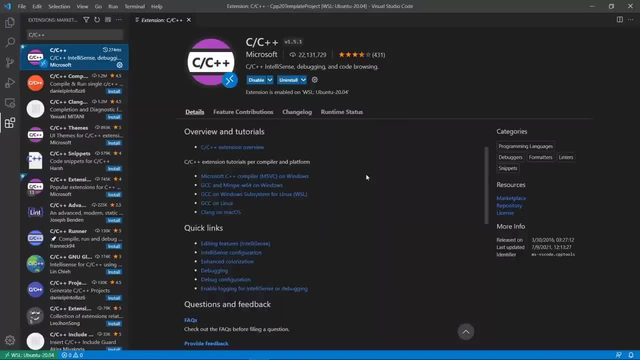 In this lecture. In the next one I will try and show you How to set up a Visual Studio Code To use the compilers that we installed In the last lecture, And meet me there. In this lecture I am going to try and show you. 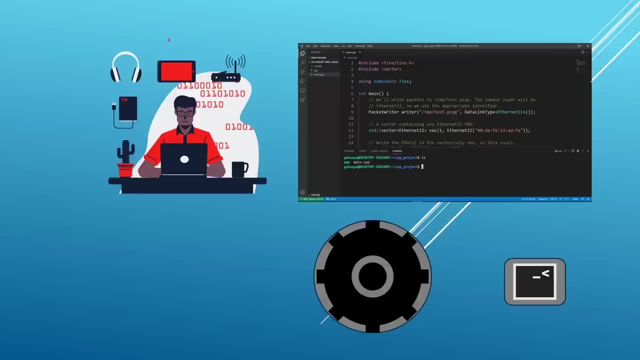 How to configure Visual Studio Code To use the compilers That we installed on our Mac system In a previous lecture. So we want Visual Studio Code To be able to pick up our GCC compiler And use it. We want it to pick up our Clang compiler. 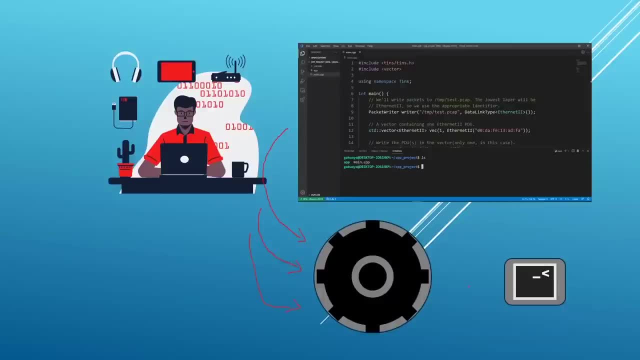 And use it. We also want it to pick up our Clang compiler From Apple and use it to build binaries That we can then run on our system here. So let's see how to do this. I have to say I don't own a Mac device. 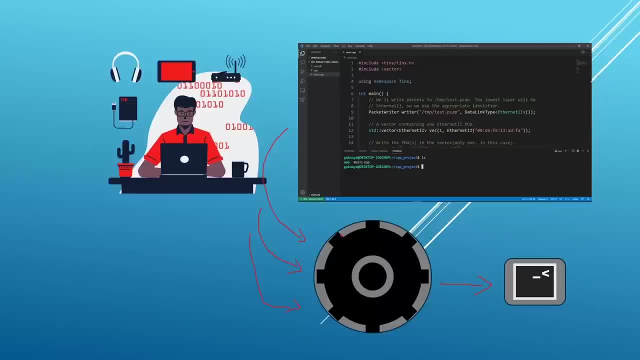 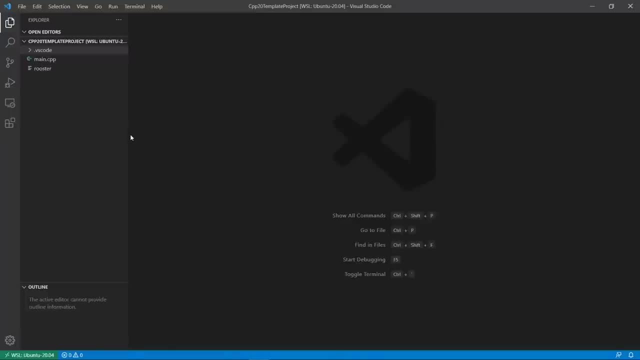 So the best I can do here Is describe the process to you And if you have a problem You can tell me. I will do the best I can to help you out. Okay, so once you have Visual Studio Code installed, You are going to create a folder somewhere. 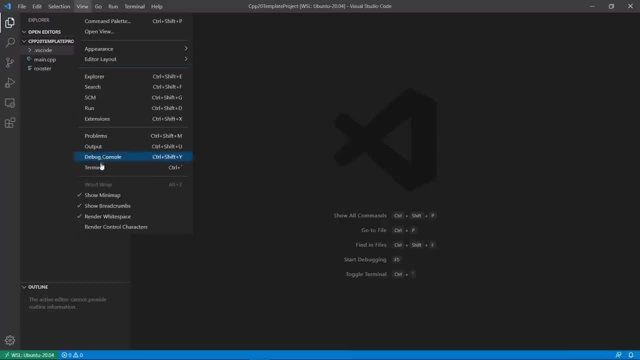 And open Visual Studio Code from that folder, And what you will basically do Is use the terminal To navigate to a location. You are going to create a folder. You can even call it CPP template project. You are going to hop over into that folder. 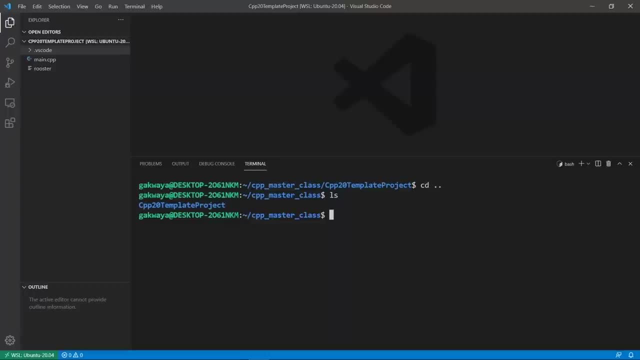 And then open Visual Studio Code from that folder here. So for example, We can hop over into CPP And run code And say dot, That's going to open Visual Studio Code in that folder And from that folder You will create a main CPP file. 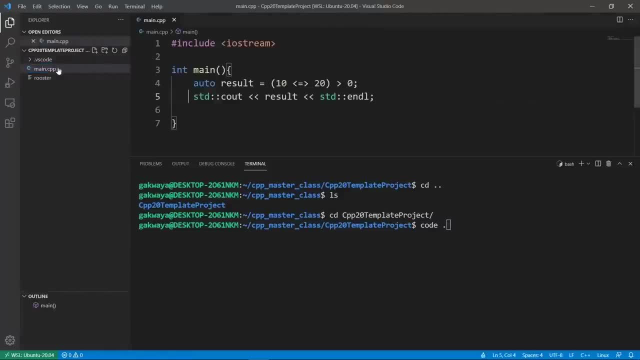 By clicking on the plus button here And you will create a CPP file- Call it main CPP- And you can put in the content here. And once you have this, The next task Is going to be to set up a compiler To build this little thing. 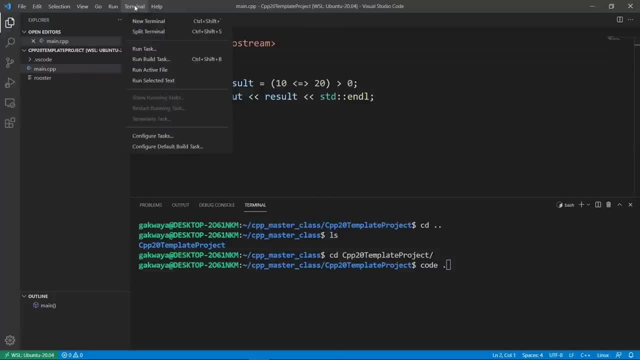 So once you have this project, You will come to terminal- I think there is going to be a terminal menu somewhere- And you will choose, configure tasks. Once you do that, Visual Studio Code is smart enough To scan your system And find any compiler you have installed. 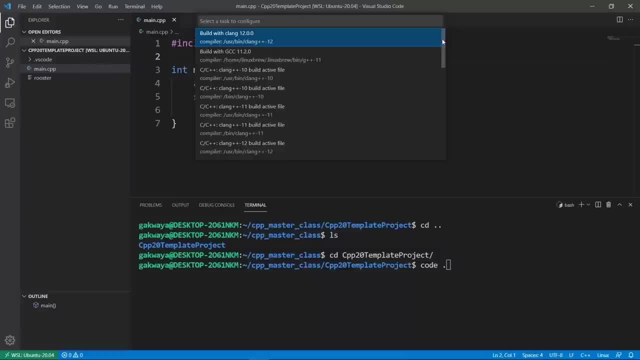 The first thing that is likely to be found Is the Apple Clang compiler. So you are going to find a Clang Plus plus compiler, So you can choose that For the Apple Clang compiler. We are lucky, We even have a tutorial on how to do that. 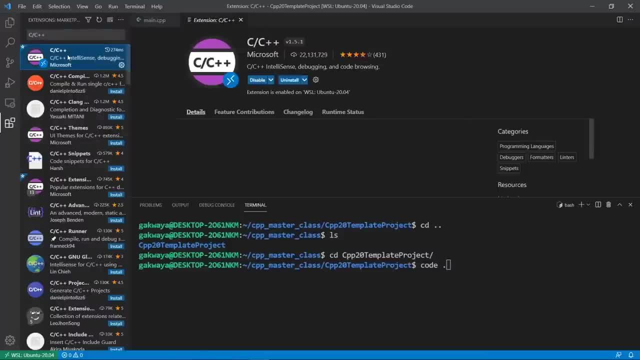 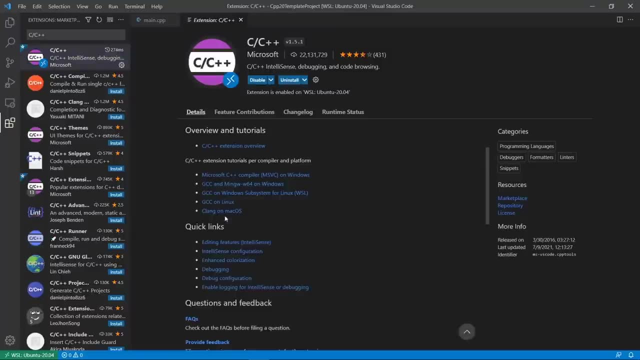 So if we click on our extensions tab here And choose our C and C++ extension, If we scroll down, We are going to see a link On using Clang on Mac OS here. This is going to give us All the instructions we need. 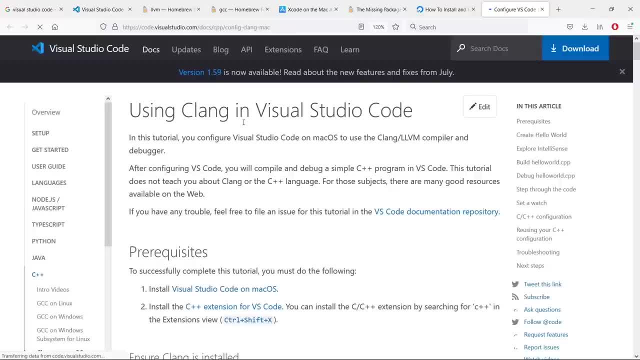 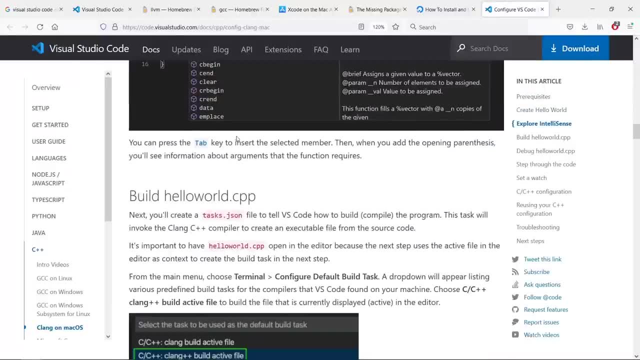 To use Visual Studio Code With the Clang compiler From the Apple company. So if you scroll down, You are going to be able to read up on all this, But what I really want you to see Is the configuration file. You are going to see that it is going to be using the Clang compiler. 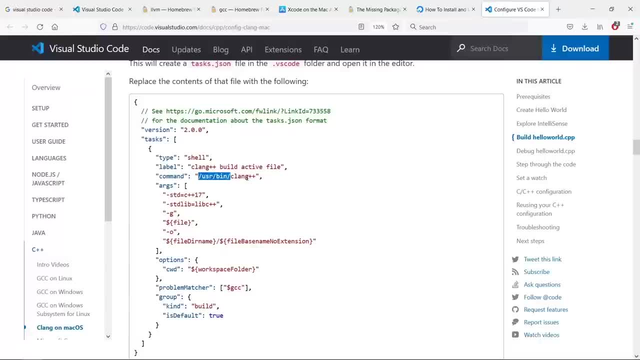 From the user bin directory And this is mostly going to be The Clang version From the Apple company, And sometimes you don't want this. So if you want to use the Clang version That we installed through Homebrew, I think you will need to go through. 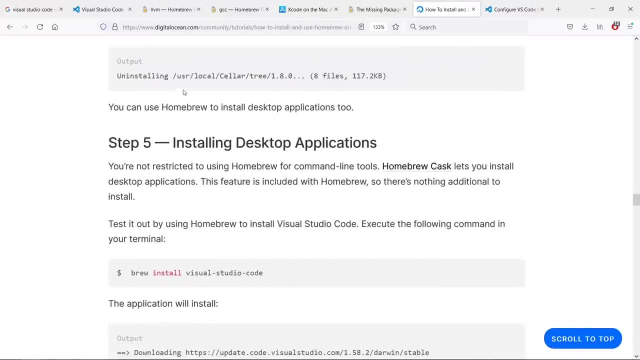 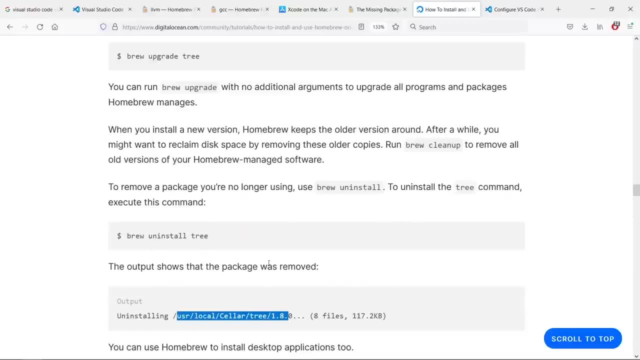 The user local directory, Because that is where Homebrew is going to put it. You are going to see that That is going to be the location here And you are going to hunt down For the Clang compiler And find your binary. 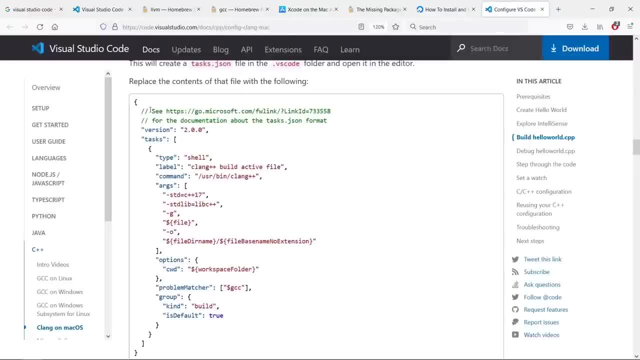 And that is what we are going to be using. next, But for the first time, If you want to use the Clang compiler from Apple, This is the configuration you need, And all you need to do in this case Is change this to C++20.. 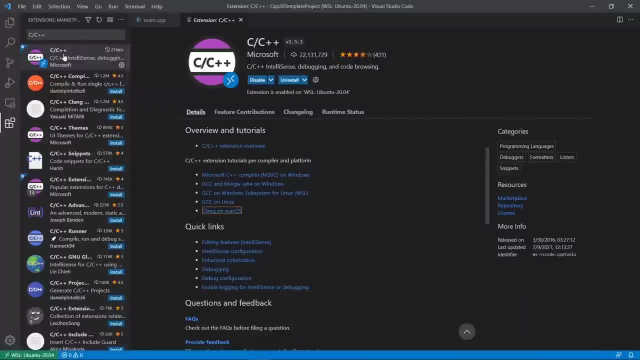 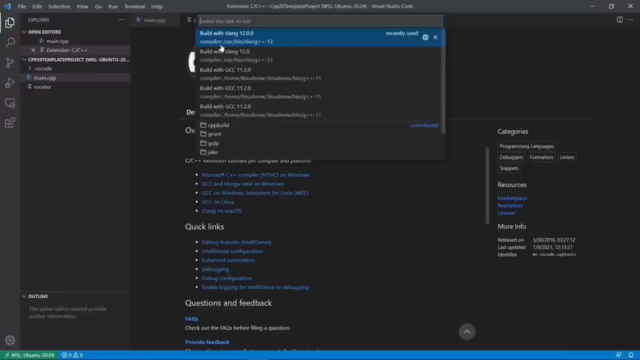 Now, once you have this configured, You will have the ability to come to terminal. Let's show our files here. You will have the ability to come to terminal And run tasks and choose the compiler- That is going to be The Clang compiler from Apple. 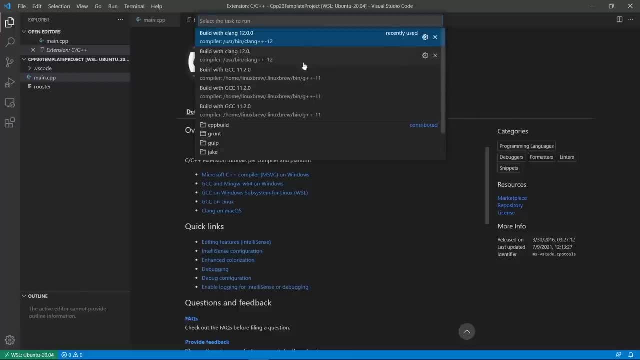 But you can also configure other compilers And all you really have to do Is choose them in the list here And you are going to have a configuration file, A tasksjson file To be exact. Let's show that up here, And that is going to give you the instructions. 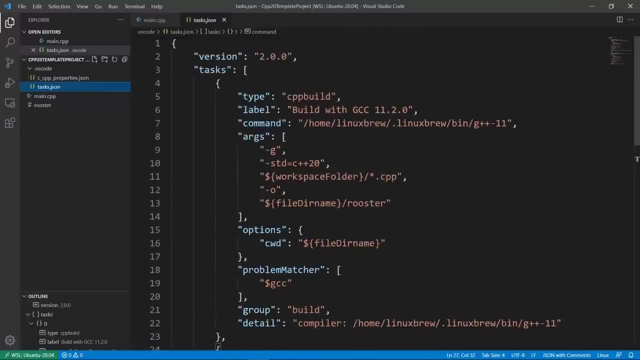 You need to build this And in most cases, You will just need to be careful About the path to the compiler. So, for example, if you are using the GCC version, You installed through Homebrew That in your location. You are going to make sure that is the correct one. 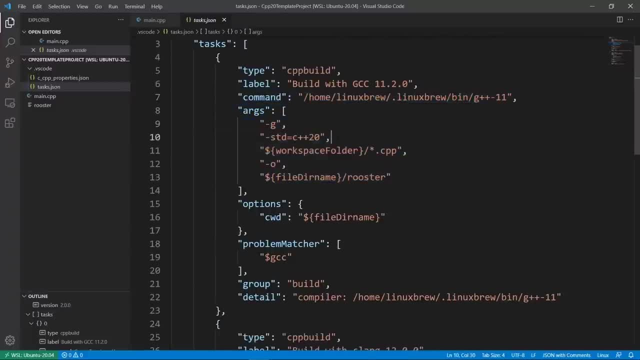 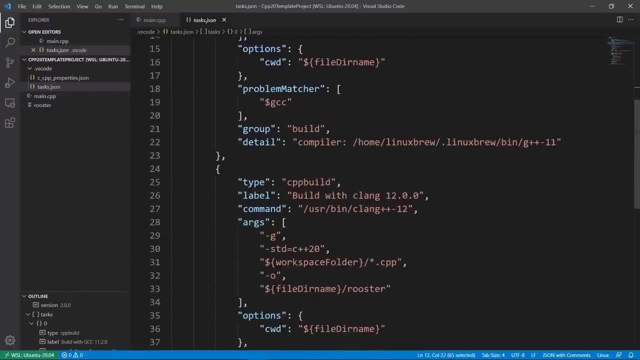 And you will put in this instructions here To tell your compiler To build every single CPP file In the directory here. This is what we do. If you use Clang, You are going to have something like this And again, I am describing this to you. 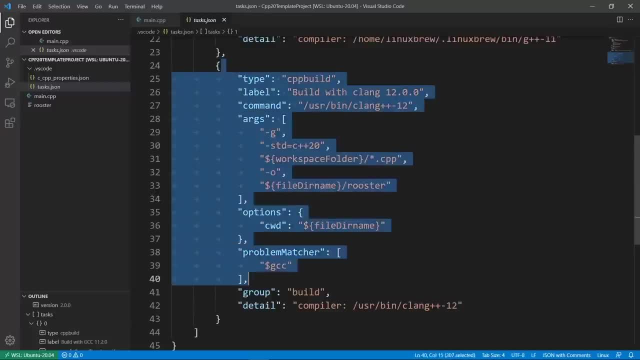 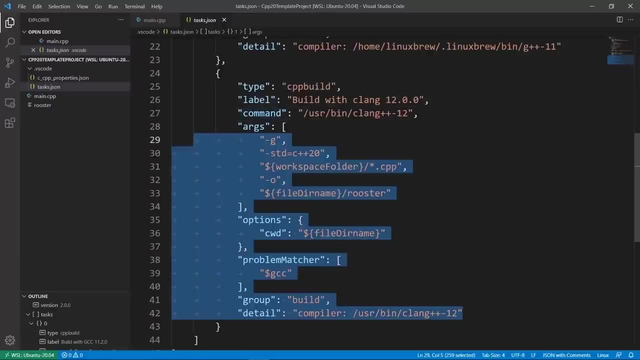 Because I don't have a Mac Available to me right now And if you have a problem, You can tell me. We can try and sort this out. If you want to use your Visual Studio Code instance And compile C++ programs, 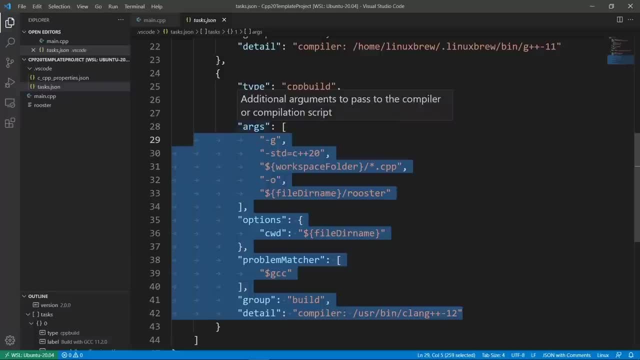 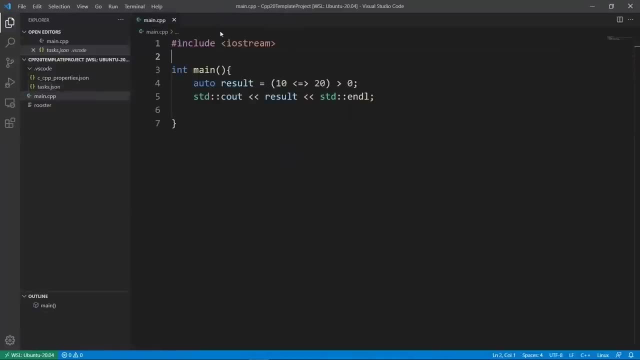 Using either the Apple Clang compiler, The LLVM Clang compiler Or the GCC compiler, And all these are going to be compiling In C++ 20 mode. Again, to build You need to make sure you have the file selected And choose whatever compiler you want to use. 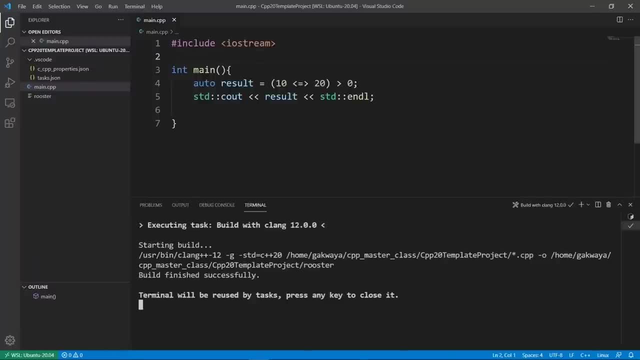 For example, if you want to use Clang 12. From Homebrew, You are going to select that And it is going to be used to build your project And you will have the ability to run your project Just like we do here. 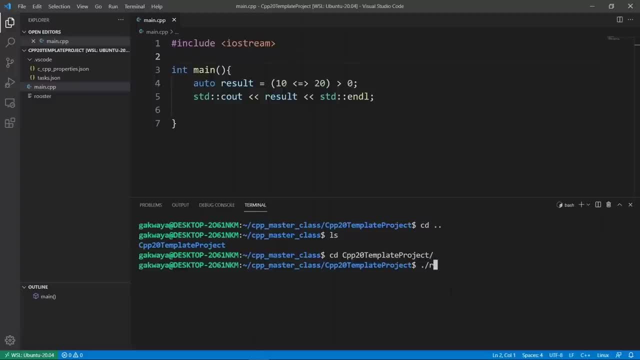 And it is going to work. Let's make sure we are running Rooster here, Our binary, And it is going to run and print a zero, And this is going to work. Again, I am really sorry I don't have a Mac device available to me. 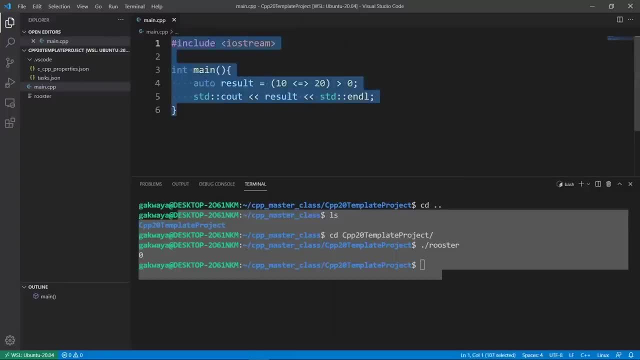 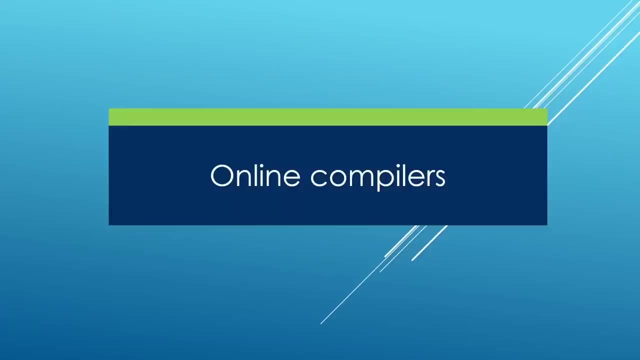 But this is what I have to work with now. If you have a problem on a Mac device, Please tell me. I will do the best I can to help you out. In this lecture, We are going to explore the option To use online compilers. 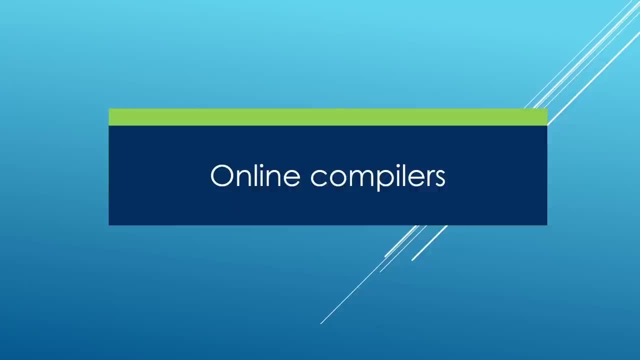 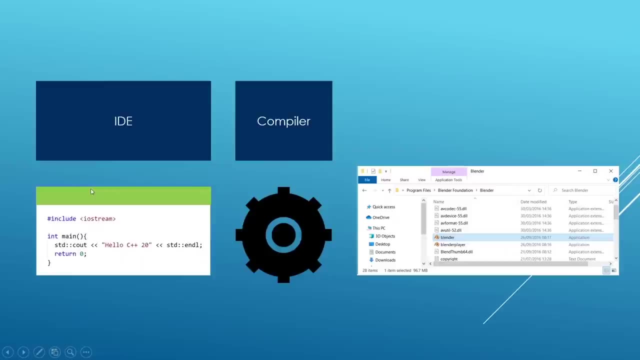 Because, for whatever reason, We can't install a radio compiler on our system. And again, the goal Is to be able to turn the code we type Into what looks like an IDE, Into a compiler, And get a binary That we can run and see the output of. 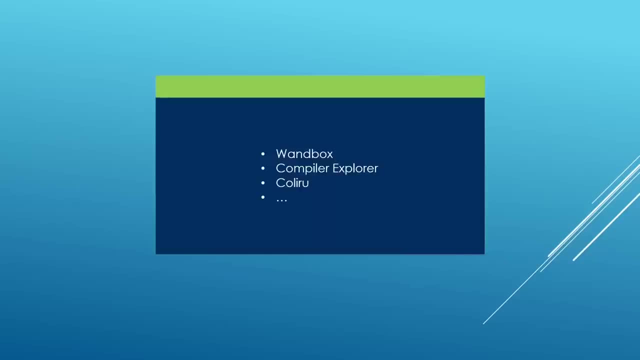 There are a few online compilers That are very popular Within the C++ community. OneBox is one of them. There is also Compiler Explorer And Coliru, But there may be other ones out there That you can research on your own. 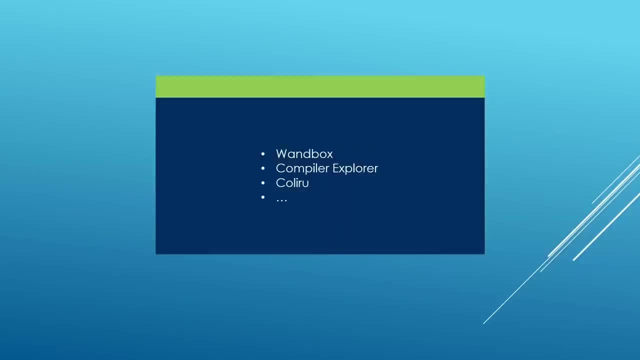 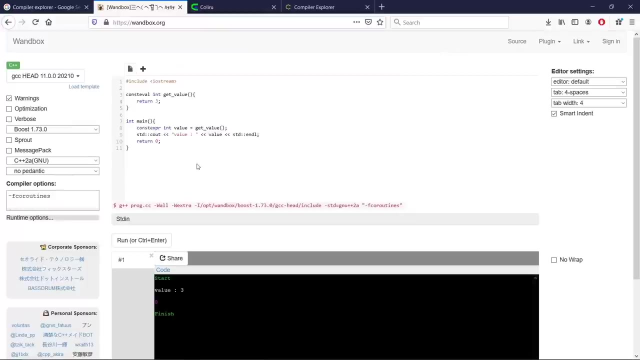 We are going to go to the browser And actually check each of these out. Okay, here we are in our browser. Here I am on oneboxorg And you see that It really looks like an IDE. Inside we have the code. 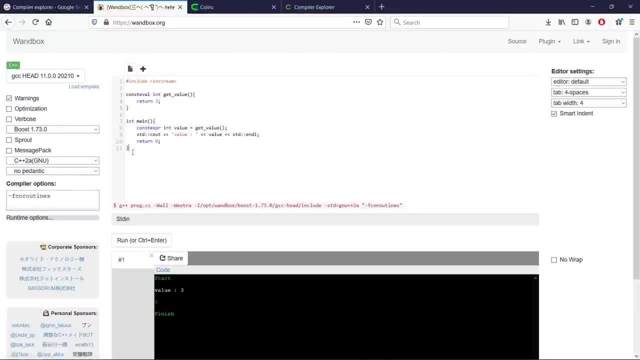 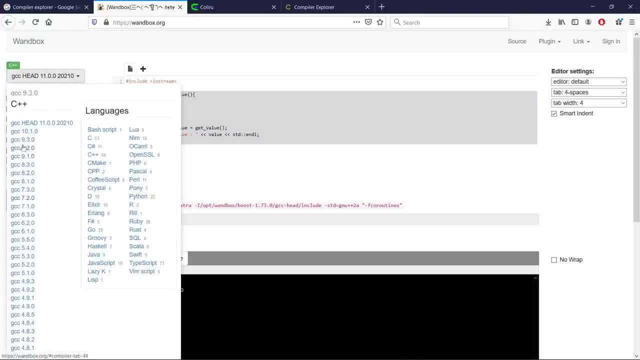 We have been running all along To make sure that it compiles With C++ 20.. On the left here we have a few options. We can select which compiler we want to use. You see that there is a couple Of GCC versions. 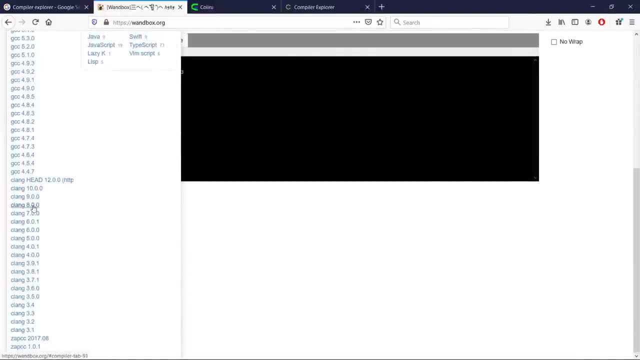 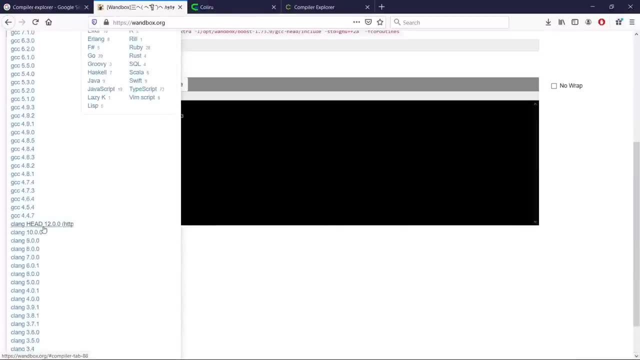 You see that this is a really nice way To test things across GCC versions. You see, we have Clang 12. So if you want to test Clang out, You can select it. Let's actually try this. So we are going to use Clang head. 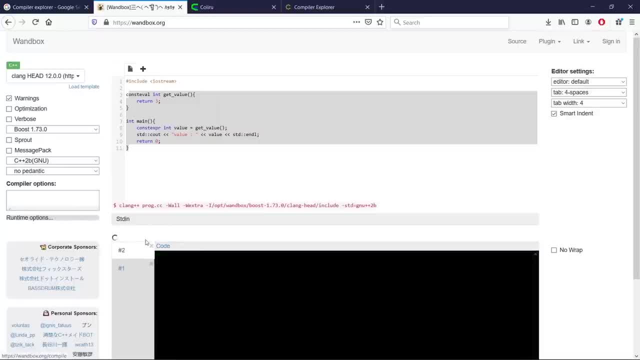 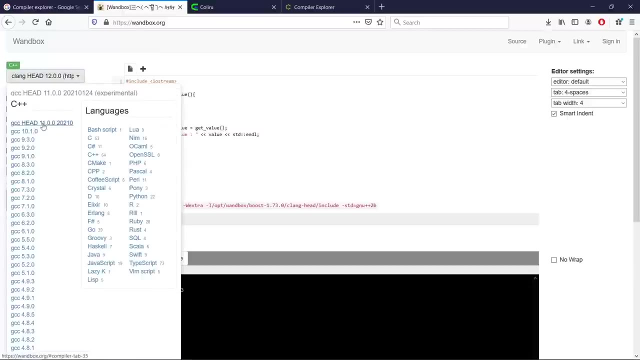 And try to compile this. So let's hit enter And see if Clang 12. Supports C++ 20.. And you see that it really works. Clang version 12. Should support C++ 20.. Like this, Let's go back to GCC. 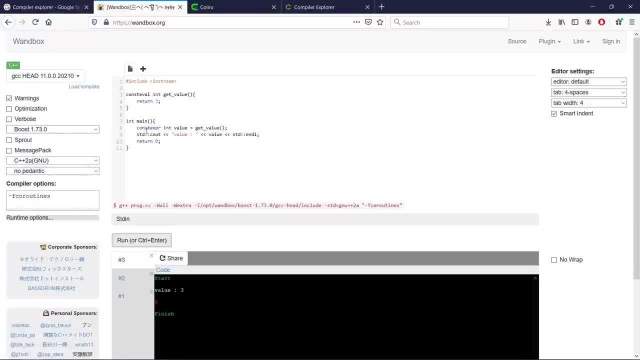 Because that's what I like, And you can try putting different things In your C++ code To see if the compiler actually responds. For example, We can say stdcl- Hello there, Stdcl, And if we run, We are going to see. 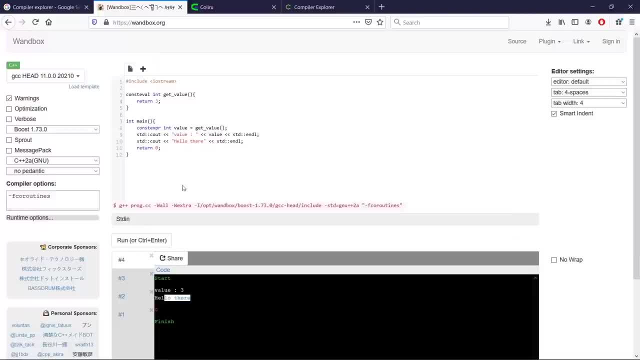 The message output here. Another good thing with these online compilers Is that you can share The code And anybody will be able to look at the code here And run it, So this is a really good way to Get help from your instructor. 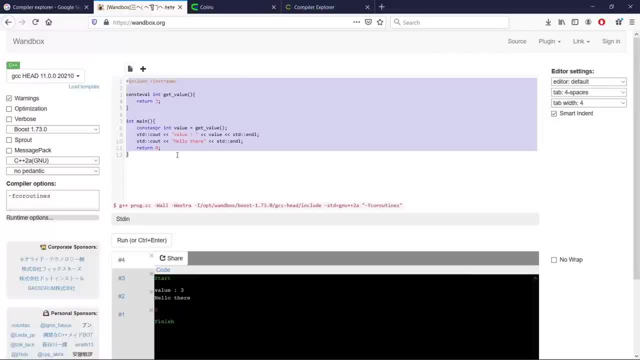 So I do encourage you: If you run into a problem, Come and use one of these compilers And send me the link. The way you can send the link: You can hit on share here, This button. here You are going to get the URL. 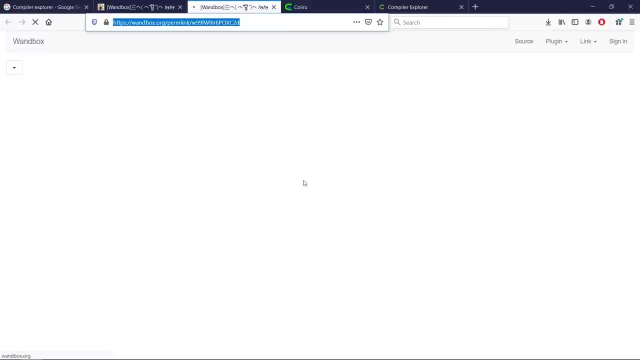 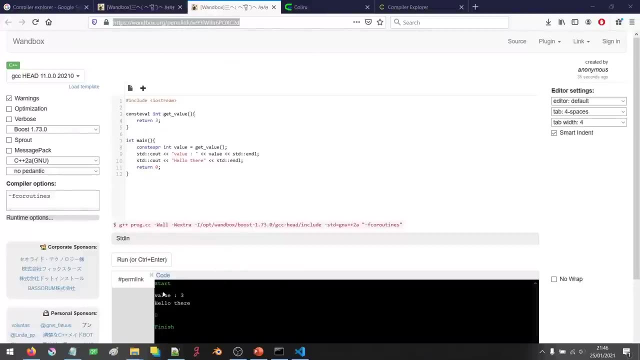 That you can copy and send to anybody, Just like we are going to see here in a minute. Okay, you see that It is the exact same thing And anybody on the internet Will be able to see your code And try to find whatever the problem is. 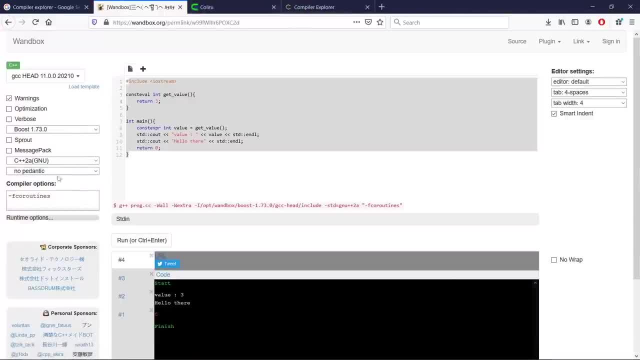 And help you out very fast. One box is one compiler. You can play with the options that we have here. You can load different libraries. You see they have a lot of boost libraries, But this is of no interest To us right now. 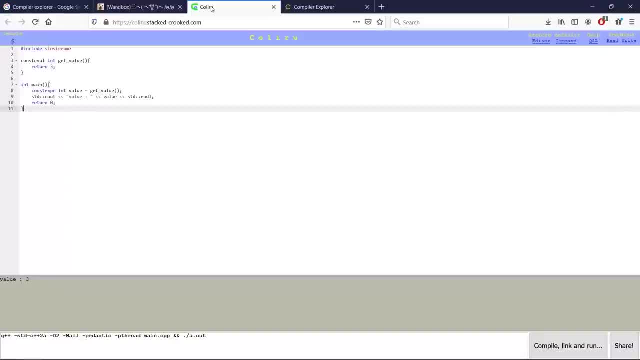 You can play with it And see what you like about it, Which is another online compiler. You see, it doesn't have a lot of options Like we had in one box. For example, you cannot change the compiler. It is going to be using G++. 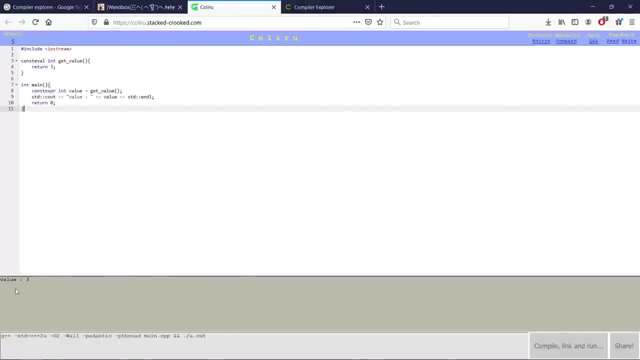 But if we hit compile, Link and run, It is going to run our code And we are going to get the output here Again, we can try and change this, So that you know I am not lying to you. So we can say stdcl. 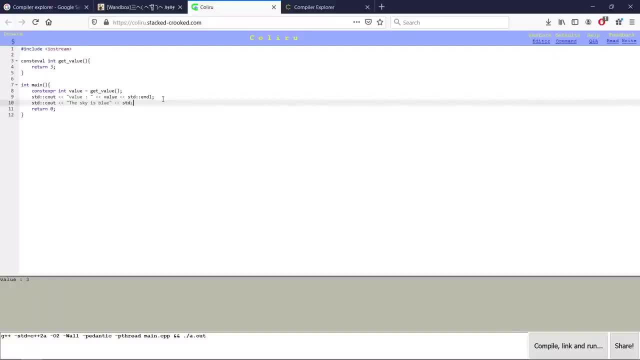 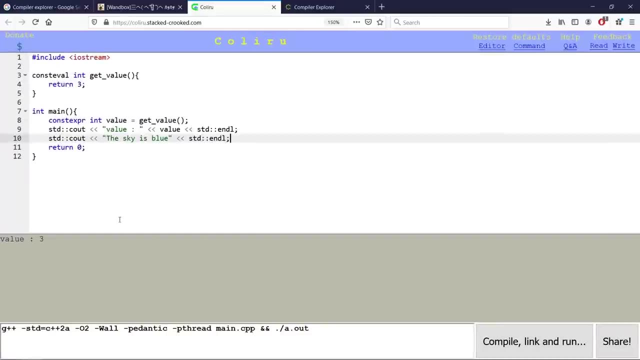 And say: the sky is blue, stdcl. If you want, You can hit ctrl plus On your browser And it is going to make this a little bigger. And if we compile, Link and run, We should see the sky is blue. 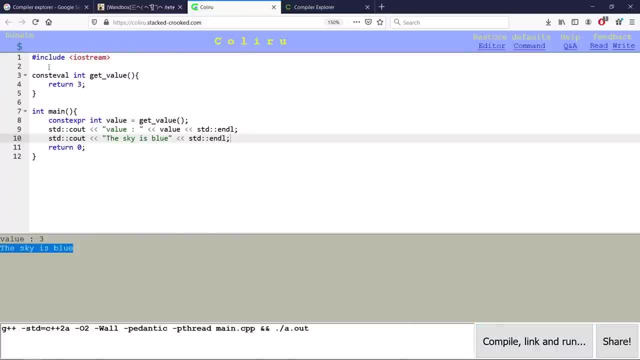 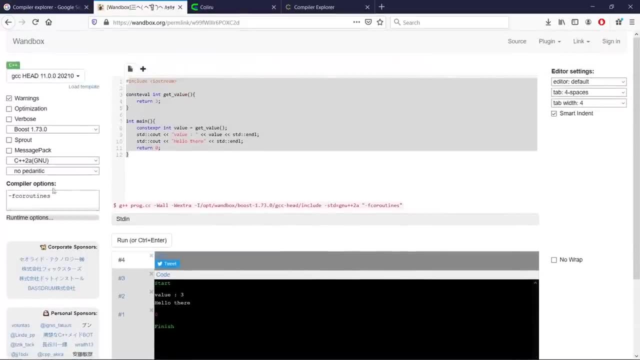 In the output window here. This is really all you can do with Coliru And if you like it, You can donate to the developers. I think we have the same thing on one box, But it is in Japanese So I can't really read this. 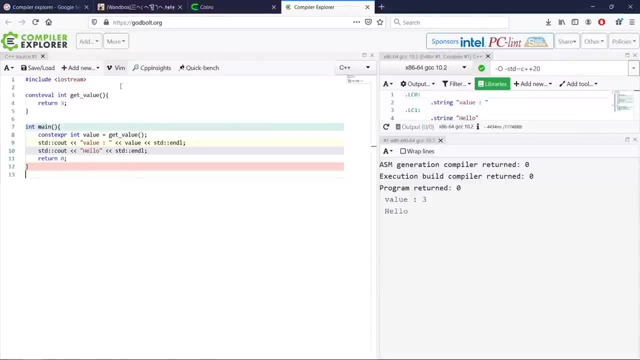 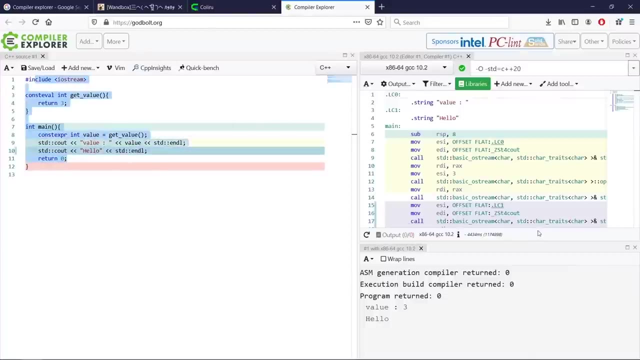 Okay, Another one is compiler explorer, Which is a really good one. The main purpose of this Is really not giving you the output. It is actually seeing assembly code That is generated For your C++ code. This is something a little bit advanced. 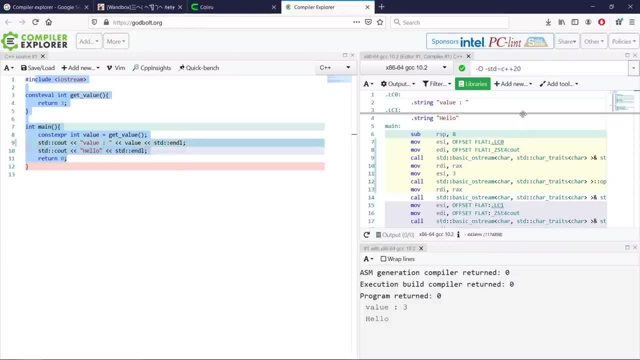 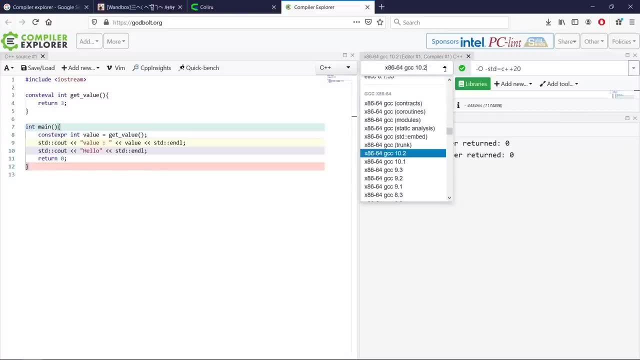 For our purposes here. So we are going to ignore this. We are just going to be using it To test our code with some of the popular compilers. If you look here On this drop box, You see that they also have a lot of compilers. 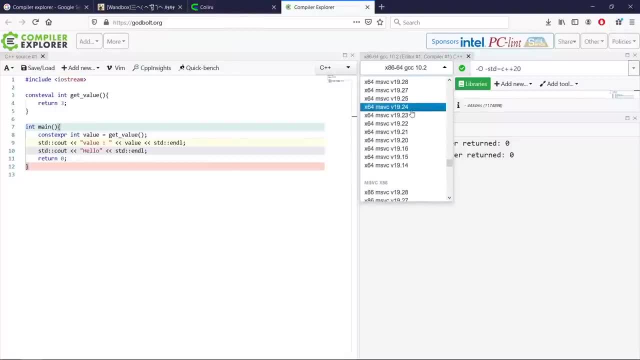 You can use different GCC compilers. They even have MSVC. How cool is this. So you can use a lot of compilers. GCC Clang- You see we have a lot of Clang compilers. We have Clang 11 here. 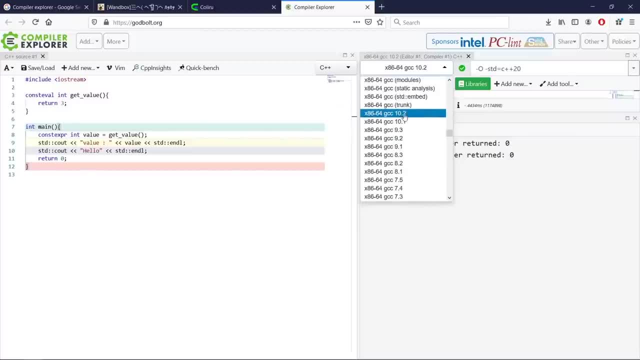 So this is a really good way To try things out. We are going to come back to GCC 10.2.. And notice that I passed The flag of C++20. To be able to support C++20. Again if I come here. 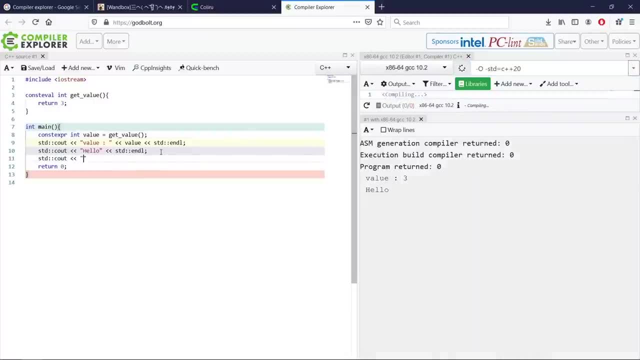 In my code and say: Cdc out. The sky is white. Don't worry about these errors, They are going to go away in a minute. Let's wait for the program to compile. You see that it is compiling. Let's wait a minute. 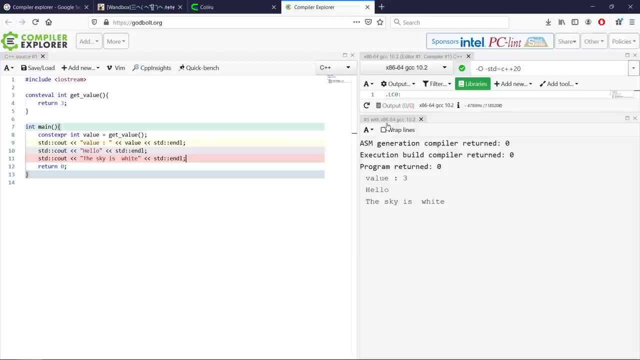 The sky is white And everything is fine. If you don't see this output here, It is possible that you didn't check this checkbox. Run the compiled output, So come to this drop box And make sure this is checked, And you should have a window. 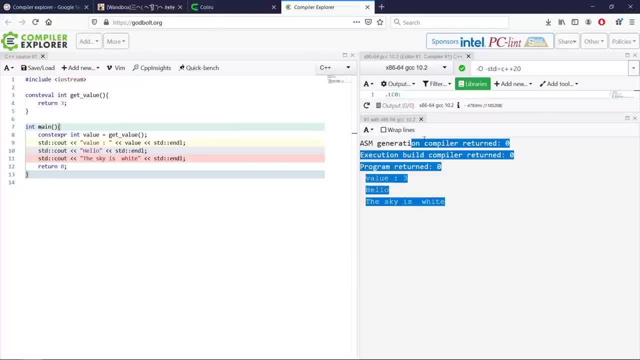 Like I have here. Compiler explorer also allows you To share your code with People on the internet. Let me see if I can find the option To share. You come to this drop box And you get a link Here that you can copy. 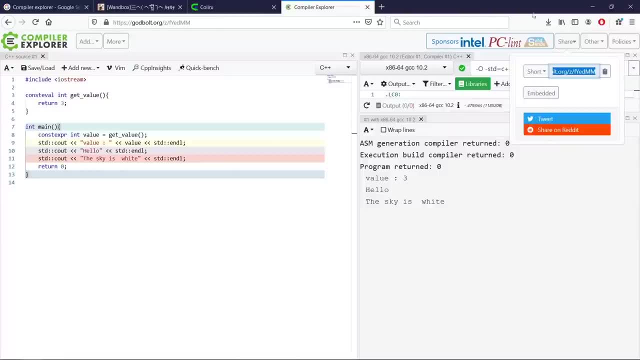 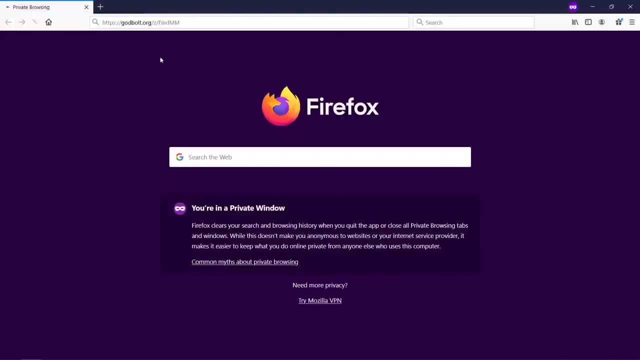 I am going to copy this And open A private window in my browser here So that we know that it is some Other browser That is going to be opening This link And getting access to the same code we have In compiler explorer. 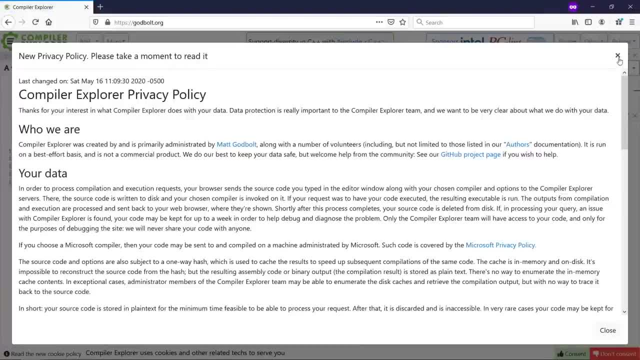 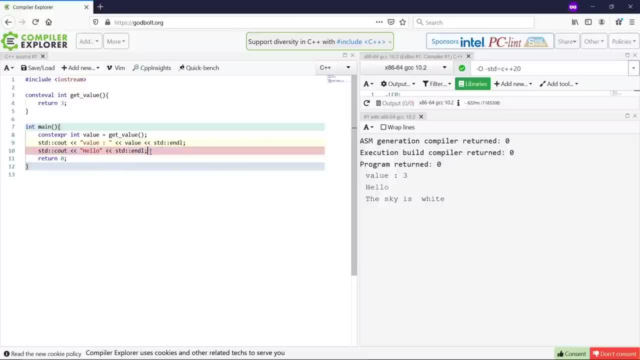 And this is going to be pretty cool. And you see that we get compiler explorer privacy. We are going to close this- And you see that we have the same code. We can try modifying this code. For example, we can take out this third line here: 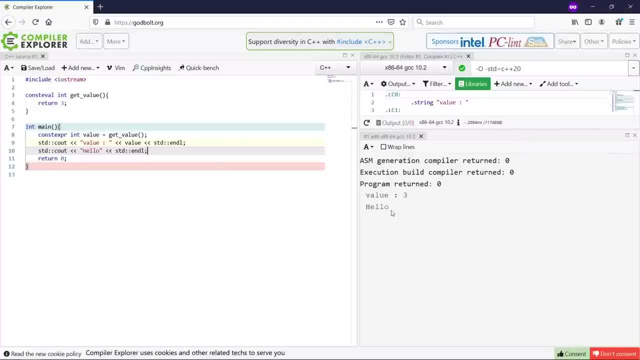 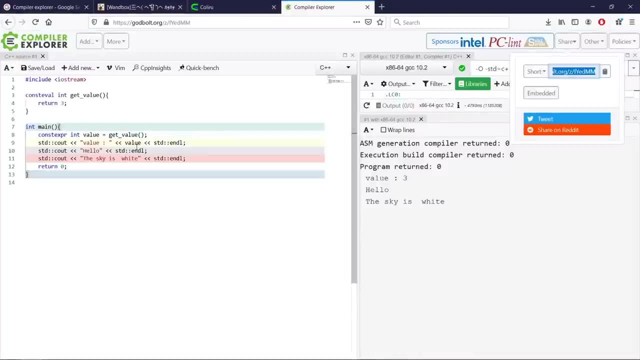 It is going to start compiling. You see that it is compiling And it is going to give us the output That we expect from this, So this is a really good tool to try out If you want to share your code With some people that are not close to you. 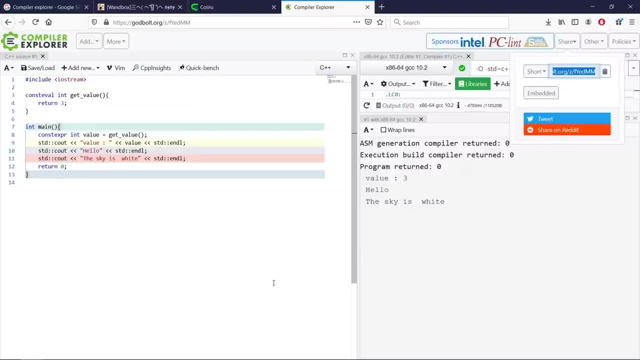 This is a really good way to do this. It is also good To try out different compilers. For example, if you don't have A GCC compiler, You can try it out here And see if it does things. For example, we didn't install clang on our system. 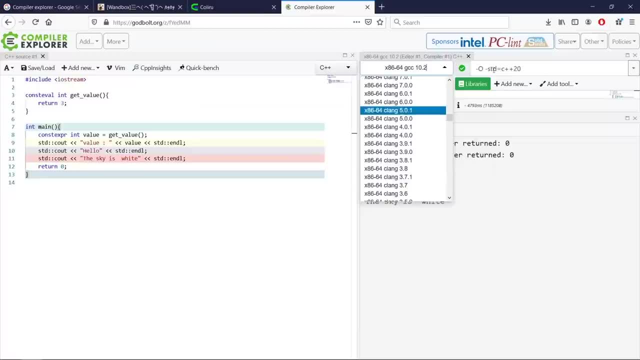 But we can try it out And see if it runs our code. But make sure you pass the correct flats here, Because you are responsible for this. If you pass the flats That don't work, You are going to get errors. For example, if we say hello here. 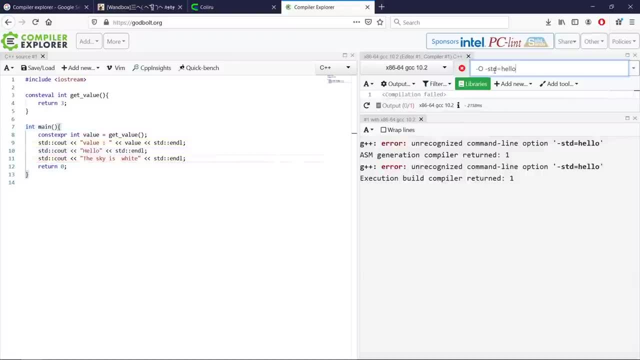 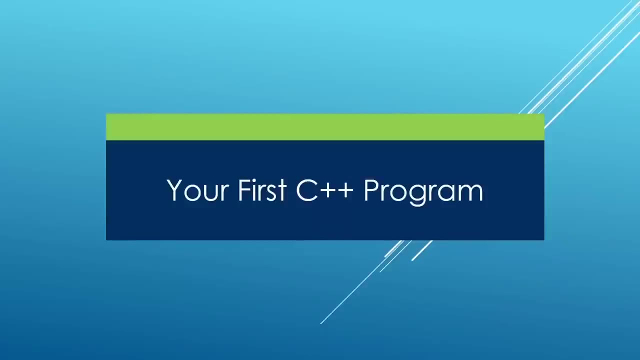 You are going to get Weird errors And recognize command line Option std- hello. But if we say C++, 20. It is going to work. So make sure you pass the correct options In this lecture. You are going to write your first. 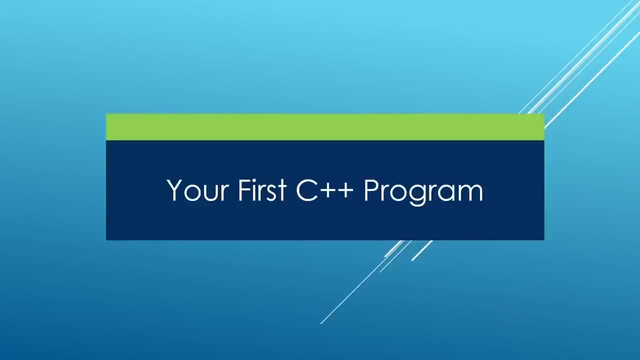 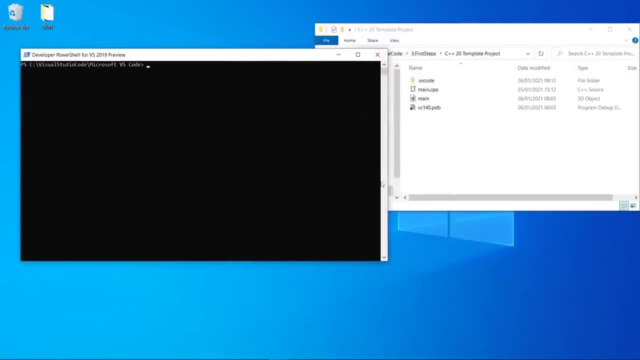 C++ 20 program And we are going to start and attempt To understand our program And actually do that. The first thing we want to do Is to set up our code So that we can open that In visual studio code. 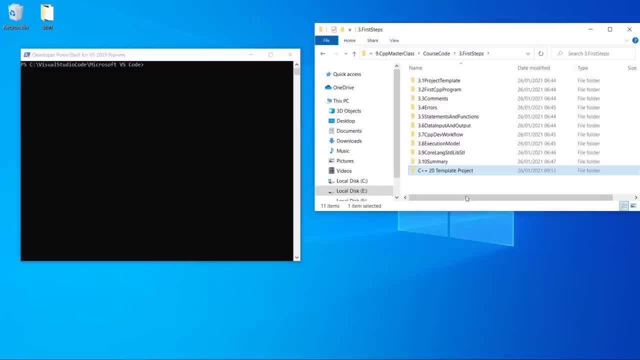 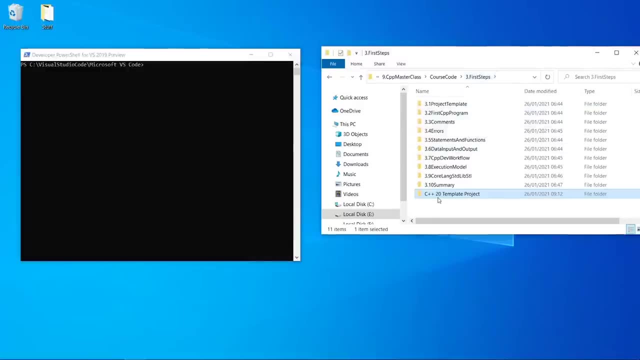 We are going to start from our C++ 20 template project That we set up in the last lecture, And I am going to be doing the projects For this chapter in this folder here. So we are going to do Our very first C++ program. 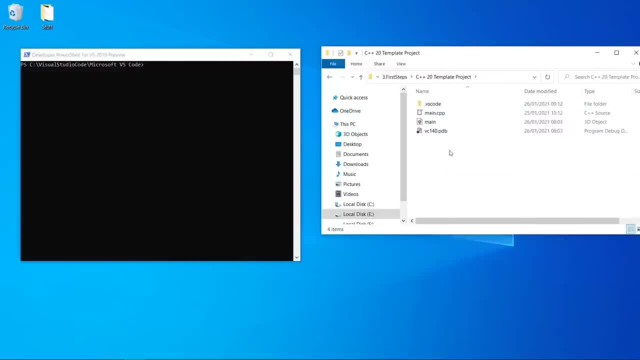 So what we are going to do Is go inside our C++ 20. Template project And I noticed that We actually left in the boiled files We don't want. So what we are going to do Is remove this main file. 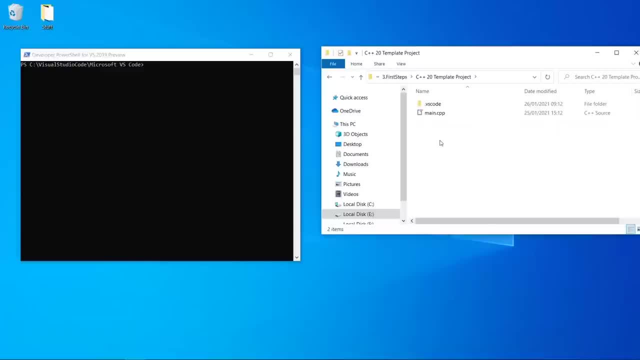 And this vc 140 thing. We don't want these here And we are going to copy The main cpp file And the dot vs code folder. We are going to copy these things And we are going to put them In our first C++ program folder. 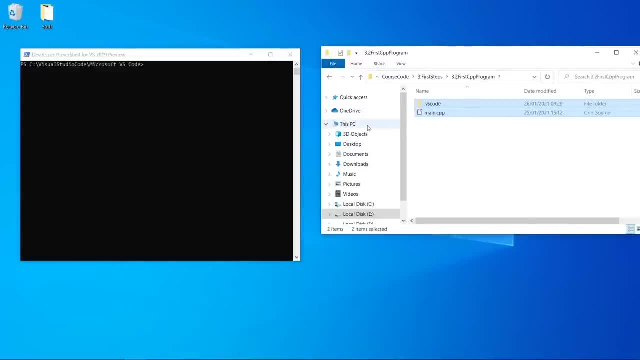 And we are going to open this folder In visual studio code. Visual studio code is not opened up. You see that I have my developer powershell opened. If you want, you can open Visual studio code directly Without going through this. 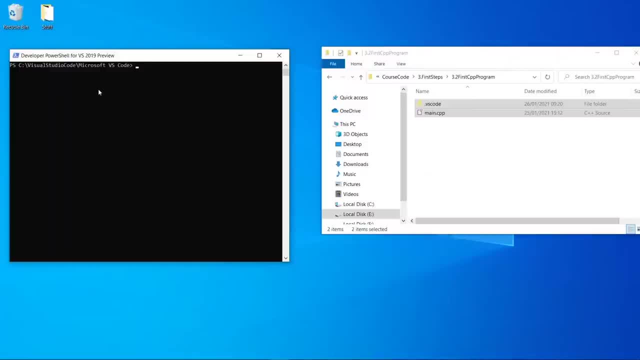 If you are not going to be using the visual studio compiler. But I want to have the option To use that compiler. So this is how I am going to open My visual studio code instance. I am going to type codeexe To open this up. 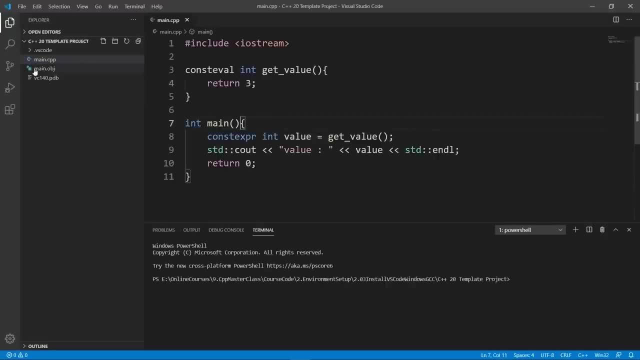 I am going to hit enter And the visual studio code is going to open, And it is going to open whatever we did in the last lecture. We don't want this project Because this is a template project From the last chapter. We are going to close this folder. 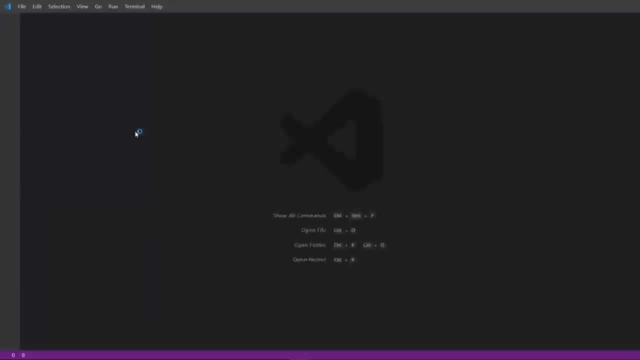 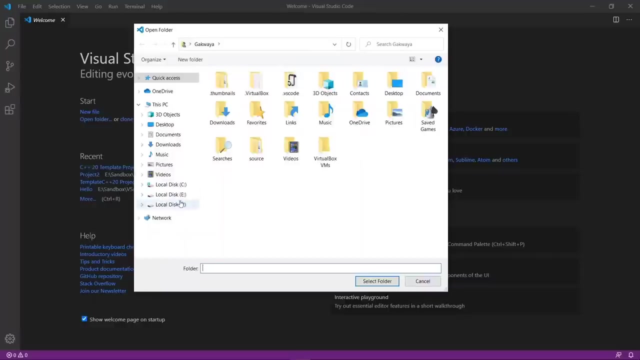 Go to file And hit close folder And we are going to open the new folder We want to work in. We are going to go to file And hit open folder. We are going to go to the location where our project is. 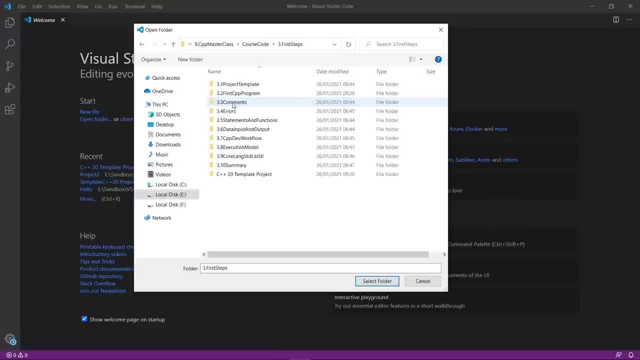 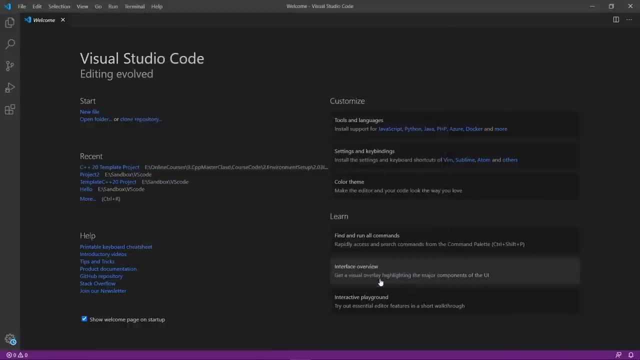 So you are going to go where yours is And I am going to go In the current chapter And choose 3.2. First C++ program. I am going to select the folder It is going to open up And you are going to see that our settings from. 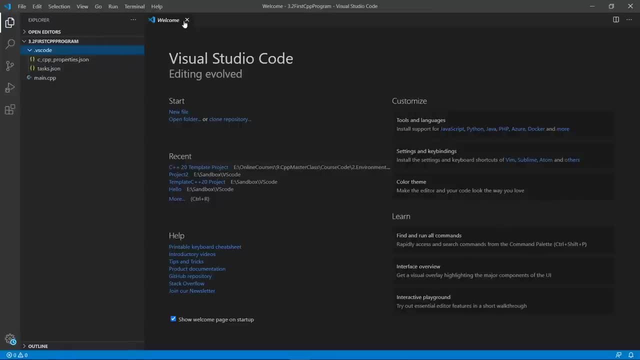 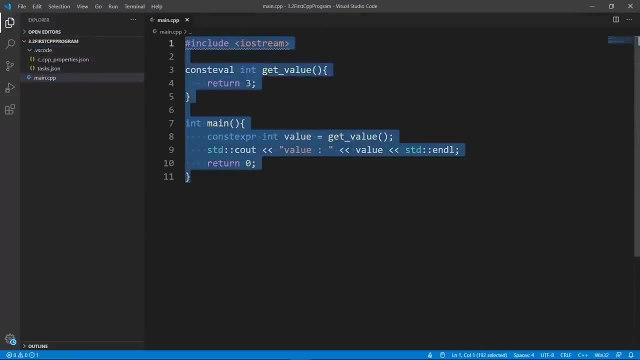 The last template project Are still Valid here. They were copied over. If we open the main CPP file, It is going to be the main thing we had in the last lecture. So we have the option to run task. You are going to see that. 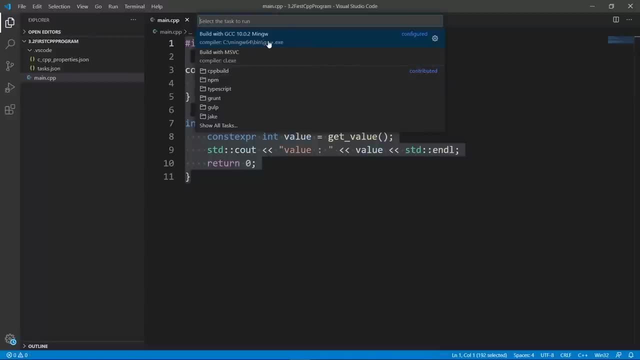 Two compilers available And this is really good. We are ready to start using this. Let's try and build this with GCC And we are going to have Our binary created. We can click in the terminal here And if we want, 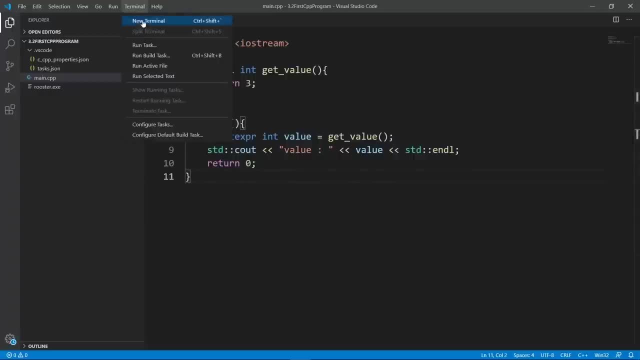 To open the terminal again. We have the option to come in terminal And new terminal. This is going to open this up. If we do dir in the terminal, We are going to see our program generated. We can remove this thing here. 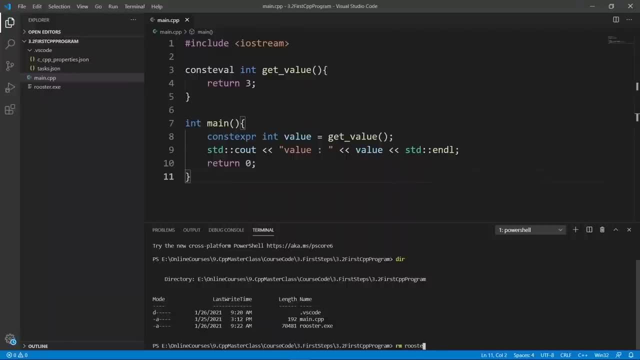 And say rmroosterexe And remove this, We can clear And we have a clean project We can start learning from. Okay, Now we have the project in. It is building successfully. Let's try to understand the code we have in here. 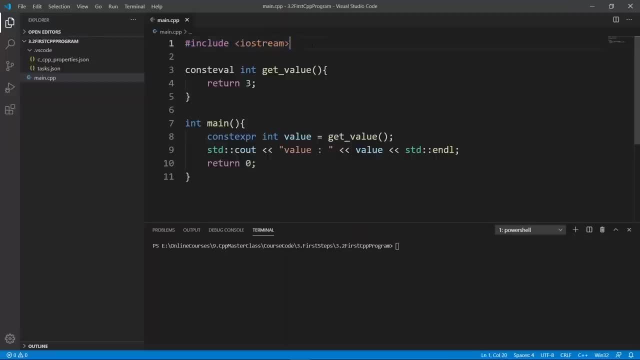 The first statement we have. It does include Iostream thing. This is a feature C++ offers To load the prebuilt libraries That we can use. Iostream is specifically Going to help us Print things to the console. We have seen that we can. 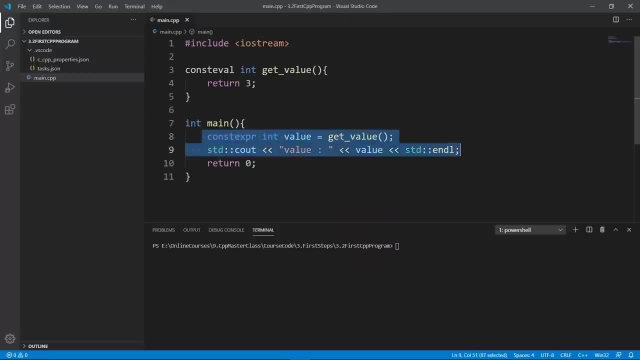 For example, print hello world. If we want, Let's take out all these things in here And say std, See how This is coming from Iostream. And we are going to put Two less than symbols. We are going to open two quotes. 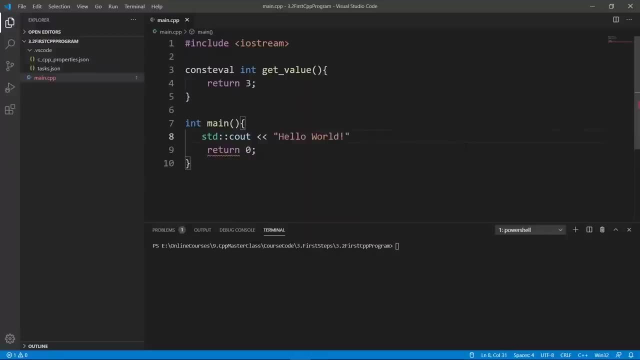 And inside we are going to type hello world. And we are going to go outside The quotes And say std, colon, colon, Endl, And put a semicolon. This is going to print things On the console If we run this program. 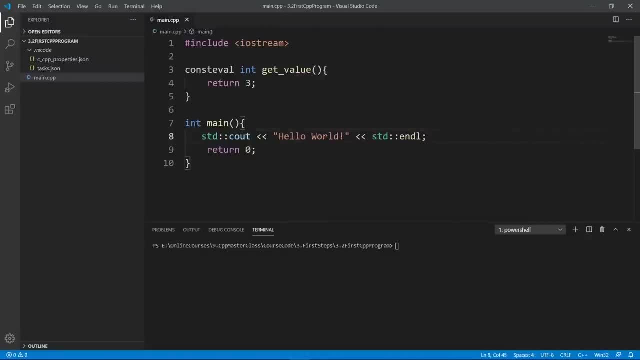 So if we run this program, The first thing we need to do Is to build this program So we can come to terminal Task- And we are going to build it with gcc- And after we have built it We can hit enter to close the terminal. 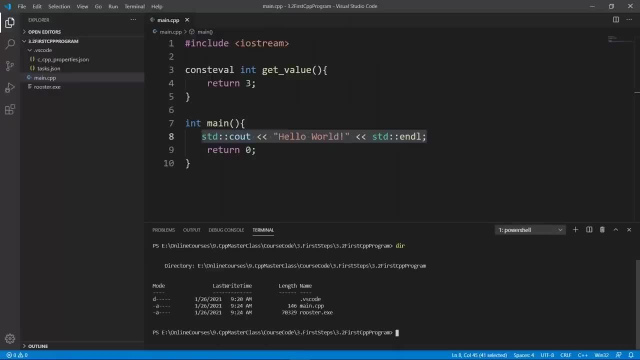 And we can do dir And in the content of the folder You see that the program has been generated. We can run it. And if we run it It is going to say: hello world. This message is coming from this statement here. 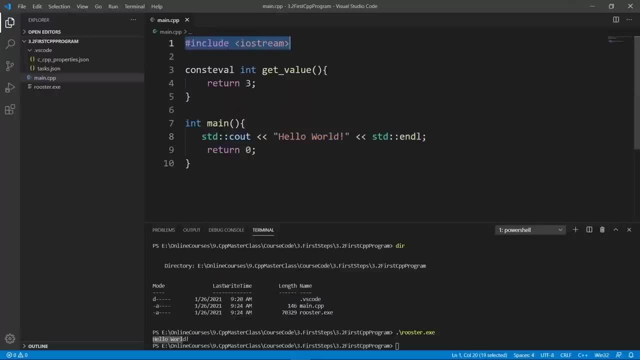 And we have this statement because We have included Iostream. To really make this super clear, We can try to remove this line That says include Iostream, And the moment we do that, You are going to see that This tab says we have problems. 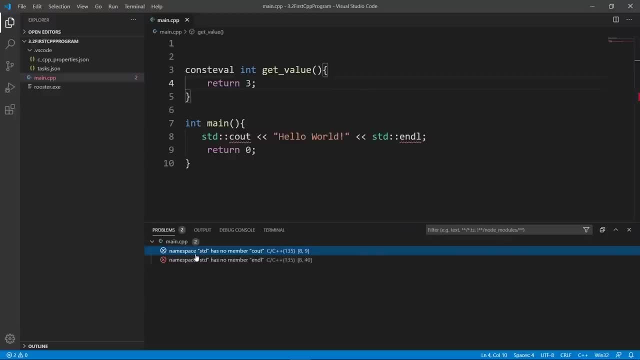 And if you open this tab You are going to see the message: Namespace SDD has no member cout. Namespace SDD has no member endl. This is because The C++ program doesn't know What SDD cout means, Because we don't have the library included. 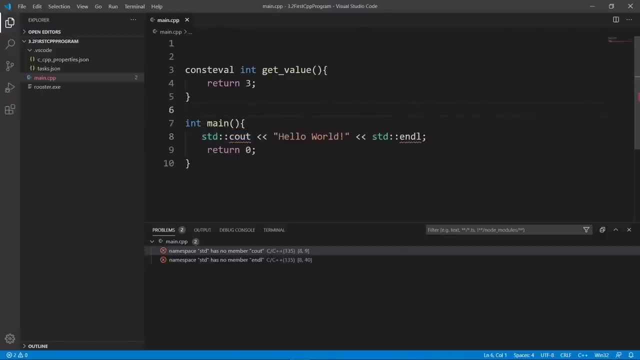 And you also see that We have these squiggly lines To make it really clear That we have a problem. So to really be able to use this, We have to include a third party library That brings these features To our program. 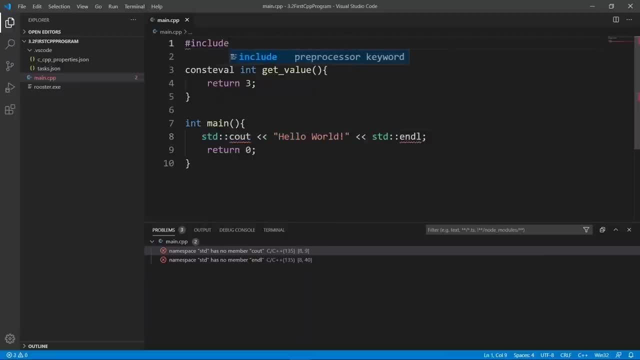 And that's what the include statement Here is really doing. So let's bring this in And we are going to say Iostream again And let's wait and see That the problem goes away. And one thing you should really know: 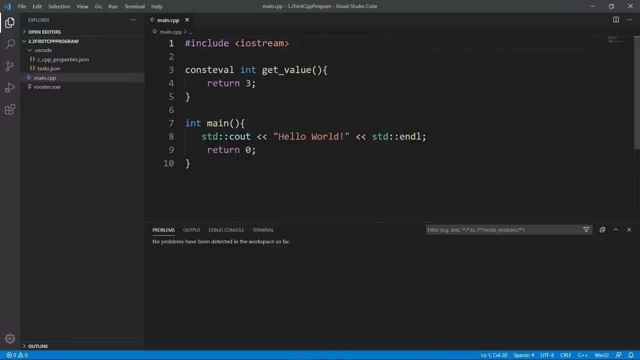 Is that we don't have a semicolon At the end of the Iostream statement. We don't need to put it there, But many C++ statements Need a semicolon at the end. Okay, So let's see here What the include statement here is doing. 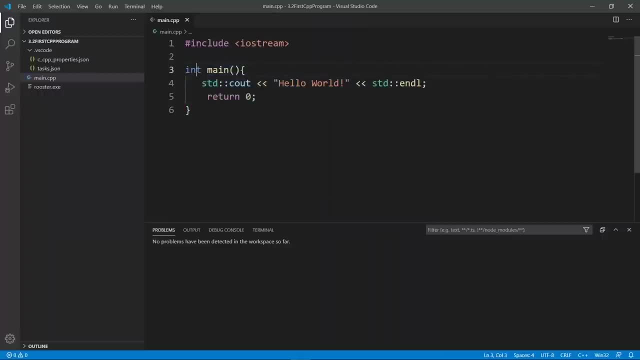 The other thing we have in our program Is this ant main Parenthesis curly braces thing. This thing here Is called the main function. A function in C++ Is a block of code That does a lot of things, But the main function here. 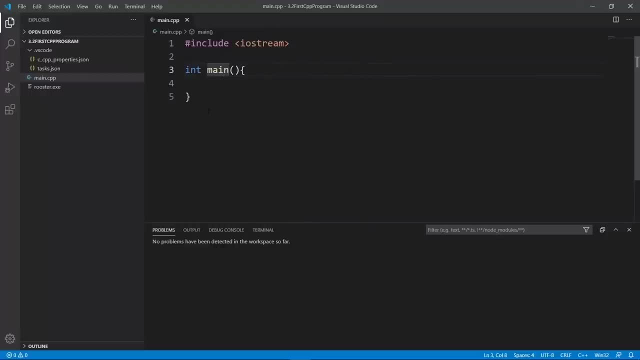 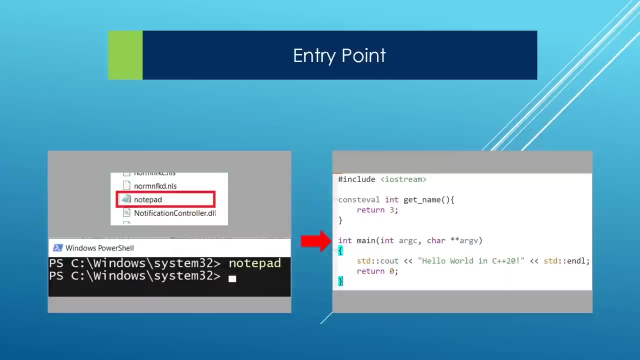 Is special Because it is the starting point Of your C++ program. We also call the main function The starting point of a C++ program, And what that means Is that if you open the program, The main function is going to be. 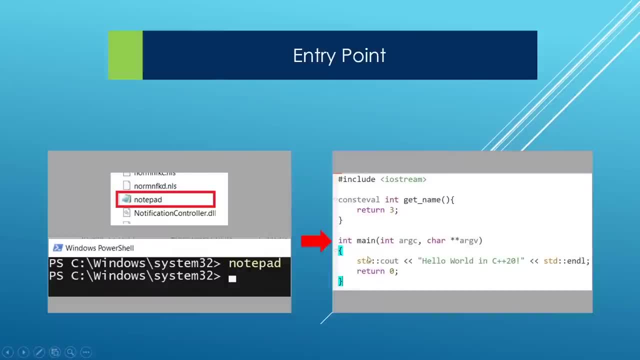 The very first thing that is going to run And things are going to be executed In the main function in order. So the statement on the top Is going to run first And the statement after that, Until we reach the end of the function. 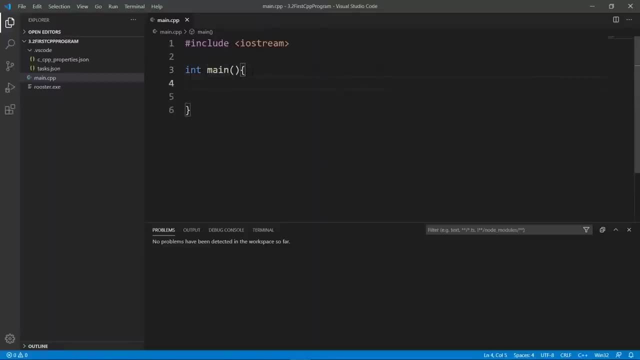 So this is what we mean here. To really drive this home, We can come here in our main function And say stdendl, Number one, And say stdendl. And, by the way, This endl statement Is going to print a new line. 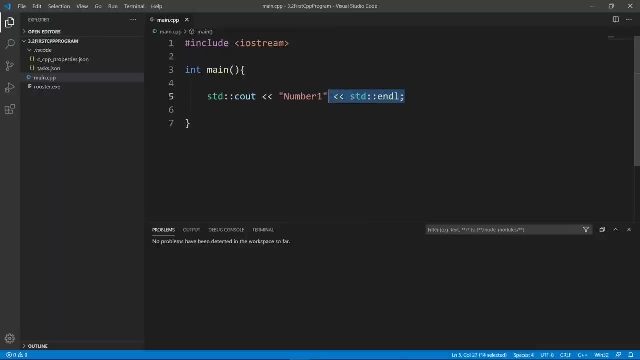 We are going to see it in effect In a moment. Let's actually take it out So that we can see its effect. We are going to also do stdcout Number two, And what this is going to do Is to print number one. 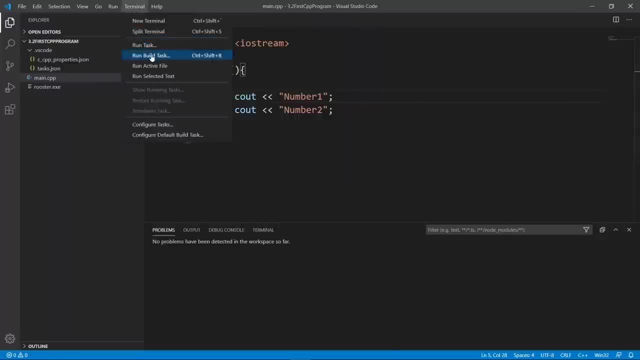 And number two. Let's build this program And if you want to build The default task, You can hit ctrl shift b For it to happen very fast. But I am always going to come here So that it is really clear. 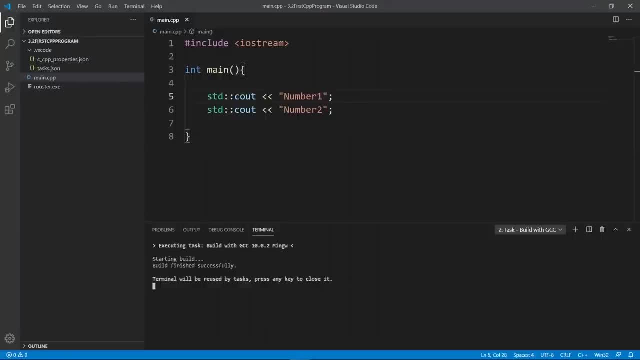 What I am doing. Our program should be generated now. If we try to run it By typing roosterexe, And again we can hit The app arrow button On our keyboard, So that's the last command that we run, And this is going to speed things up. 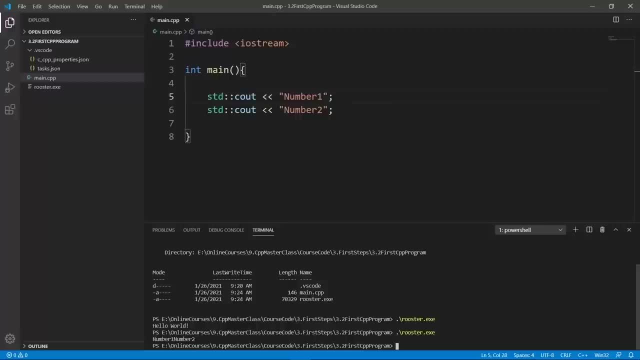 A little bit. So if we run this program, It should say number one And number two, As you see here. But these two things are cramped On one line And the reason is We are not printing new line characters After we print number one. 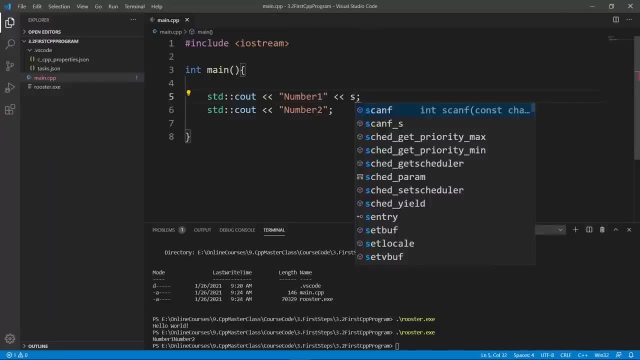 And number two, And we can solve this problem By putting in two less than symbols. This is going to put a new line character After number one. We can build again For our new changes to tech effect After we do that. 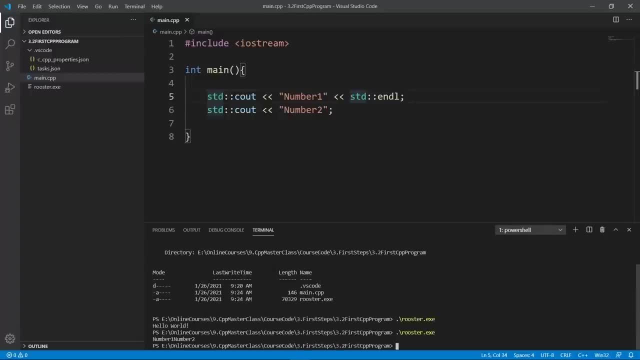 We click on the terminal, We hit enter, We hit the app arrow button. If we run, It is going to say number one And number two on two separate lines, Because we are printing a new line character After number one. I really hope this makes sense. 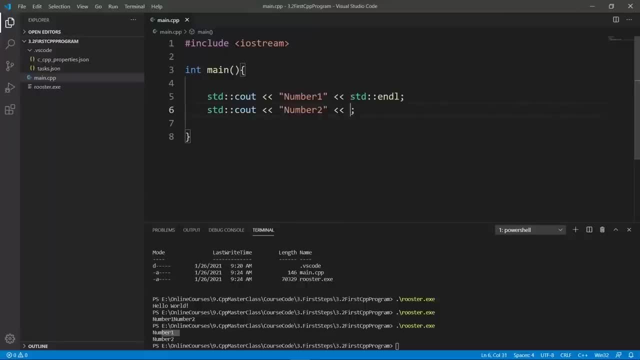 To play with us, Because if this is the first time you are doing this, Some things might not be clear, And the best way to really make sense of this Is to type code, Run it And see the effect of what you type. 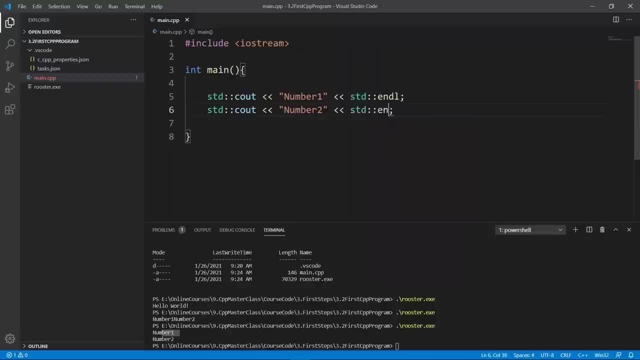 By running your program. So let's do this a couple of times. We are going to do std endl After the statement For number two. We are going to do std cl, Number three, And we are going to do std endl. 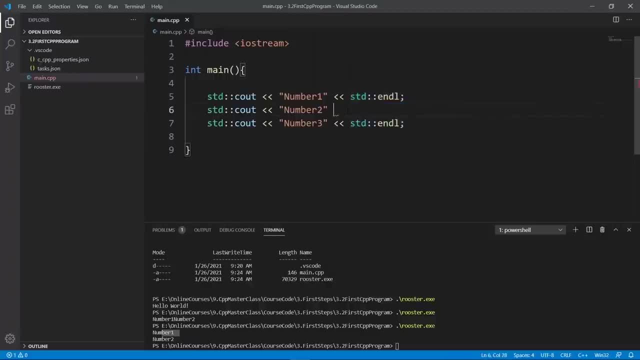 To really show the problem again: We are going to take out std endl On the number two line We are going to build. The build is going to be successful. We are going to click in the terminal: Hit enter. Hit the app arrow button. 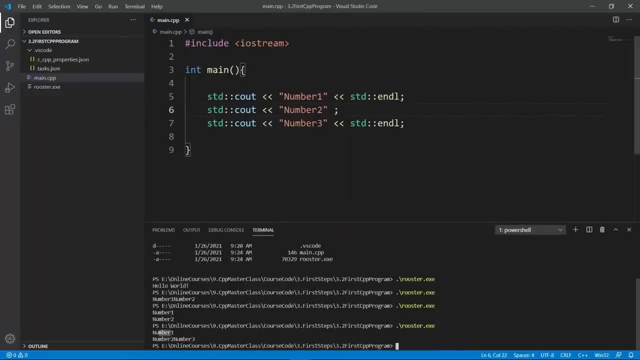 Run the program again And you are going to see it saying number one. It is going on the new line Printing number two, But we are not jumping to the new line from number two. It should be cropped on one line. That's what we see here. 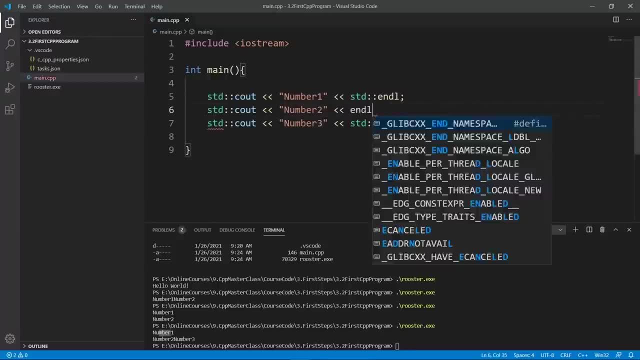 We can solve this again by putting in a new line After number two. Let's do std Endl here, And this should solve the problem. Again, let's build. We are going to run our build task. The build is going to be successful. 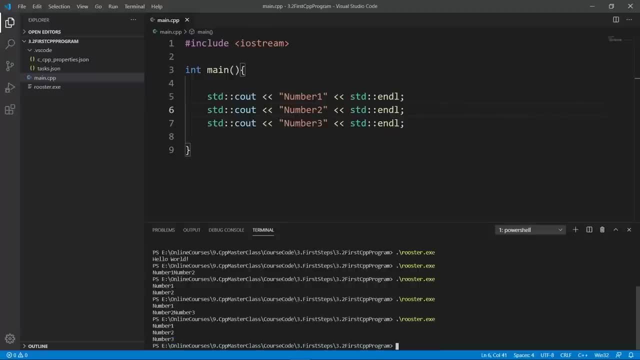 We are going to hit the app arrow to run the program. If we run it, It is going to say number one, Number two and number three. Now it should be clear That statements in the main function Are run in order From top to bottom. 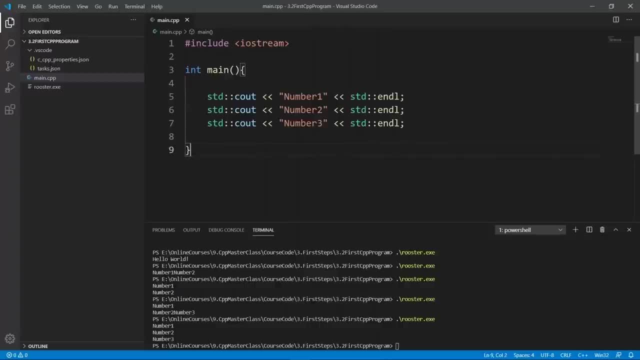 And that the program is going to end When it hits the end Of this curly brace That englobes our function. We are going to have a chance to learn more About functions in detail Later in the course, But we are just getting started. 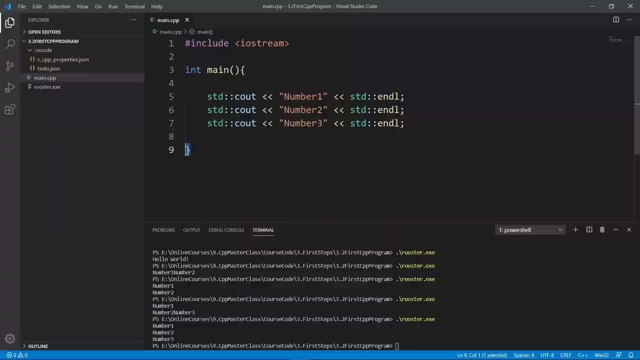 And we need to start somewhere. So that's why we are doing this main function thing here. Another thing you can do Is return from the main function, And in many examples You will see people do return zero, Something like this, And this is a way for the main function. 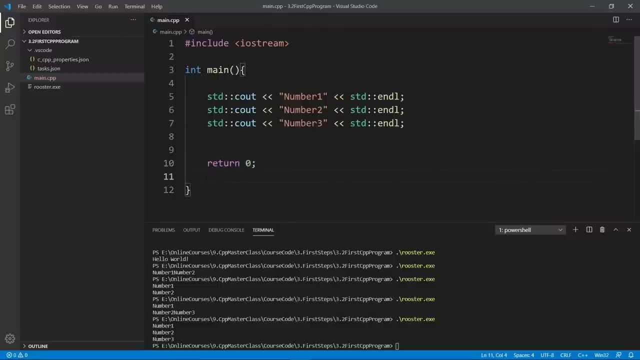 To send the message To the operating system If it finished successfully Or if there was some kind of problem. We are not going to go into Any more details about the main function, Because that's really too much For now. We are just getting started. 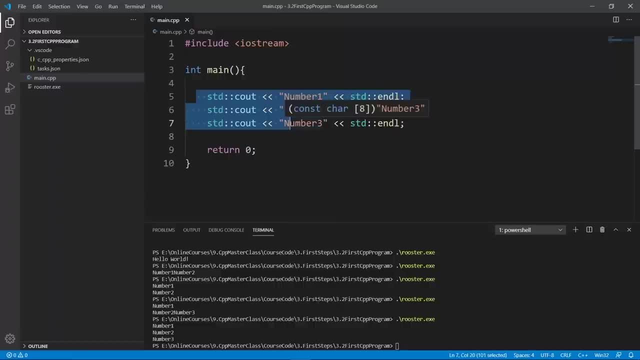 We are trying to get a feel Of how C++ works. The main message here Is really that you should be able to Print things to the console Using stdc out. You should be able to print a new line After your message. 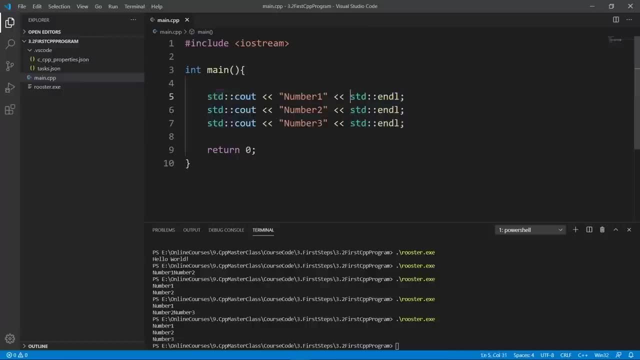 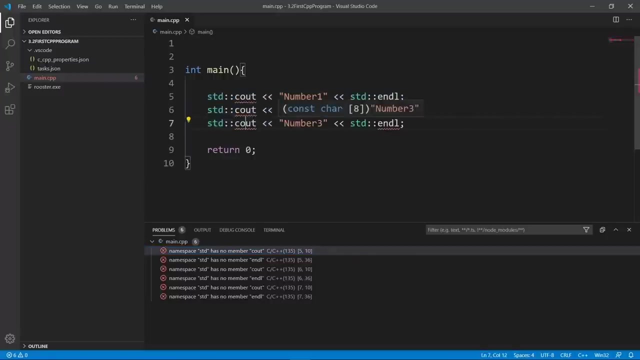 Using stdendl. This stdc out And stdendl thing Come from the iostream library That we are including here. If we don't include this library, We are going to have problems Because our C++ program Doesn't allow us to know. 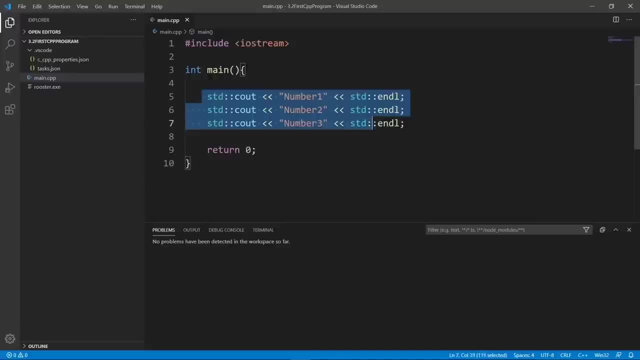 Where they are coming from. So we should really put this in If we want to use these features And we can return from a function To let the system know The operating system If the program finished up successfully Or if there was some kind of problem. 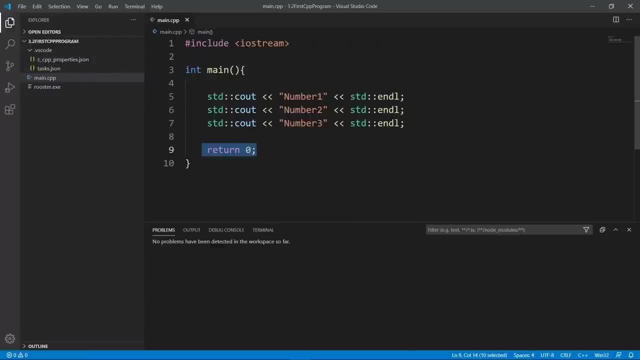 And again, this project is using The template we've done before And this is really all we set out to do In this lecture. Trying to make sense of the main function In C++, I would challenge you To write a C++ program. 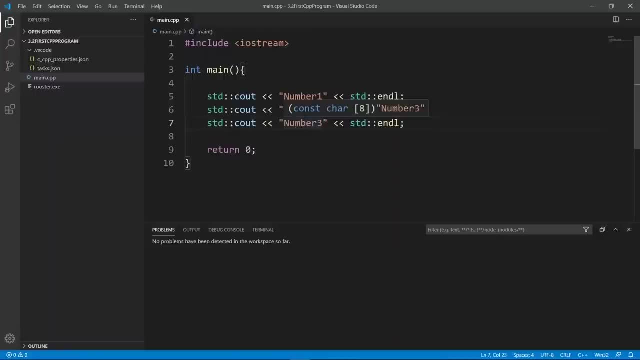 Just like this That is going to print your name 10 times. Try to do that, And if you have a problem, Please do ask me And I will do the best I can To help you out. This is really all we set out to do in this lecture. 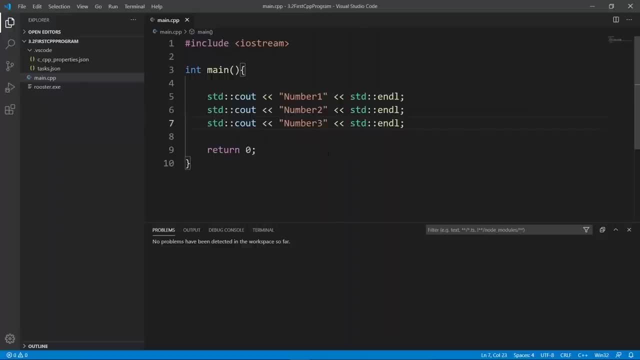 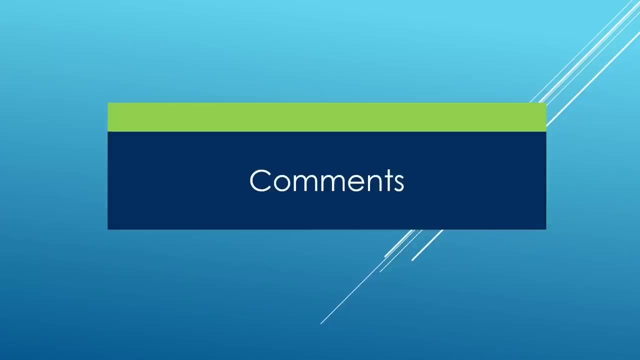 I hope you found it interesting. We are going to stop here in this lecture. In the next one we are going to start And learn about comments in C++. Go ahead and finish up here. Comments are a way To put some messages. 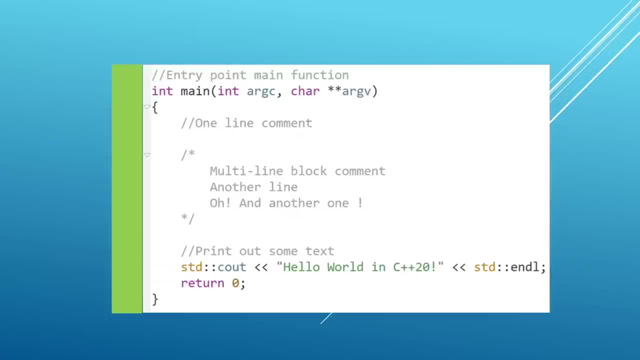 In your C++ code That are really meant To be read by humans, And one way we have to do comments in C++ Is through this backslash Backslash thing we have here. This is going to comment out the line, So the compiler is really not going to care about it. 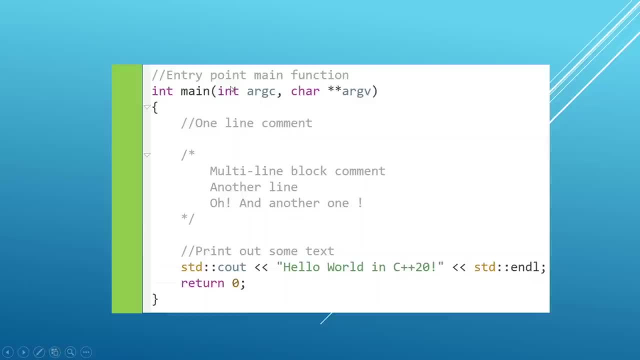 It's going to think that It is something that is meant for the developer To see. So this is a one line comment And this is how you do it in C++. You can also comment out a block of code In your C++ code. 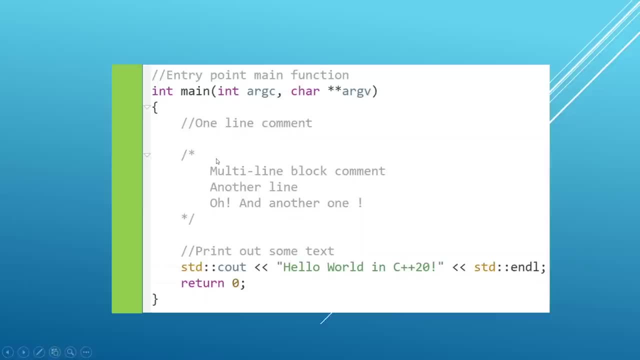 And this is something that comes in quite handy. Many times You put your comment in a backslash star And a star backslash like this: This is going to comment things out In your code And the compiler is really not going to care about this. 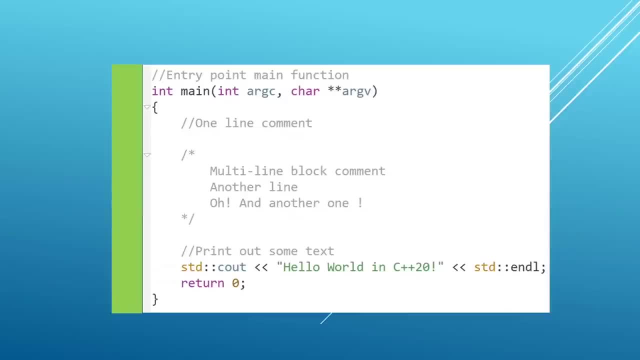 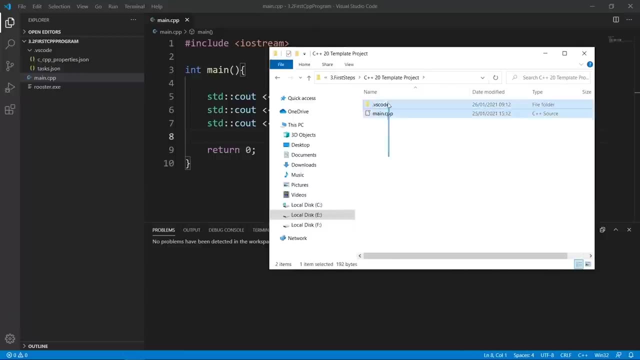 Let's hop over to Visual Studio Code And actually play with this. So here we are in the folder That is going to contain our code. The first thing I am going to do Is I am going to copy my files And I am going to go up again. 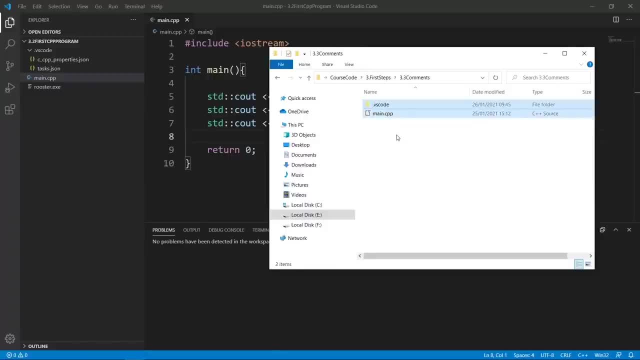 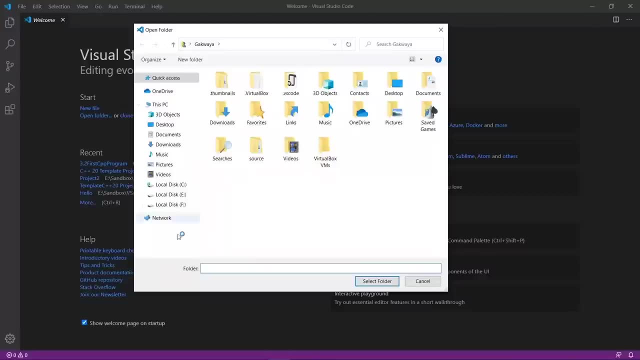 And we are going to be learning about comments, So I am going to put this in the folder On comments. I am going to close whatever folder we have opened In Visual Studio Code And I am going to browse to the location Where my project on comments is. 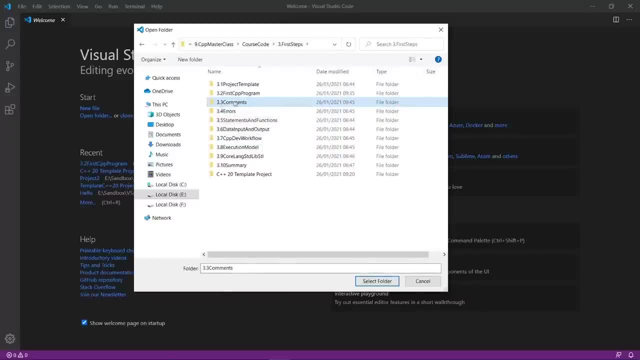 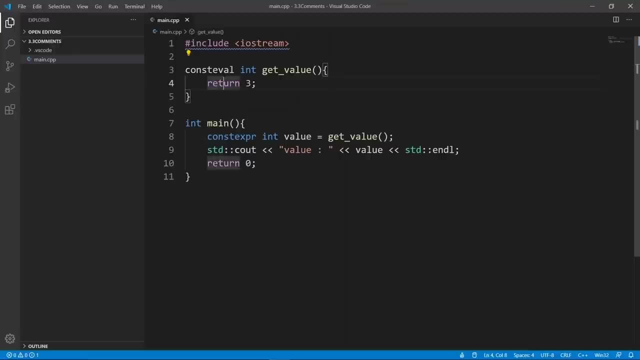 My project is in this folder That is named Three. three comments. I am going to open the folder And if I open the main CPP file I am going to find the starter project And I am going to remove this const eval thing. 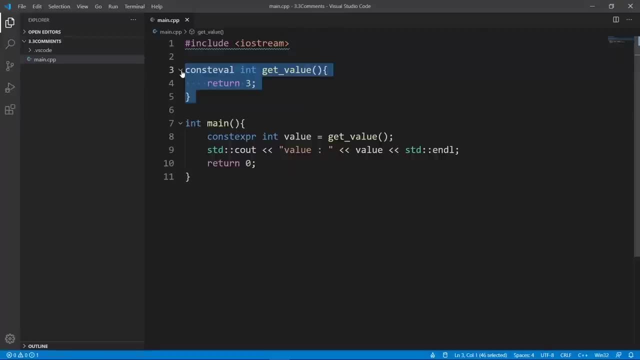 Because we are really not ready to understand this. yet It was in here to help us Test that our compilers Support C++ 20. So we are going to remove this And we are going to put in a message That says hello world. 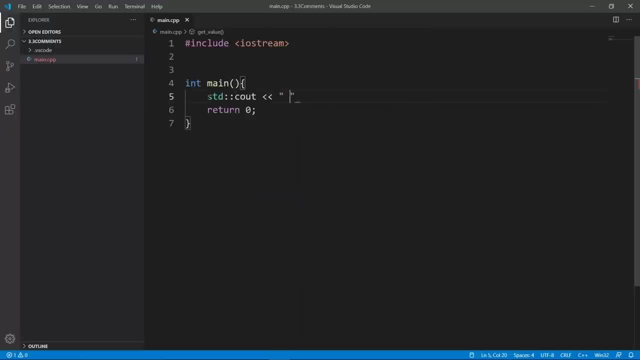 You already know how to do that From the last lecture. So we are going to say stdc out Hello world, And we are going to say stdendl. And don't forget this semicolon at the end. If you do, You are going to have problems. 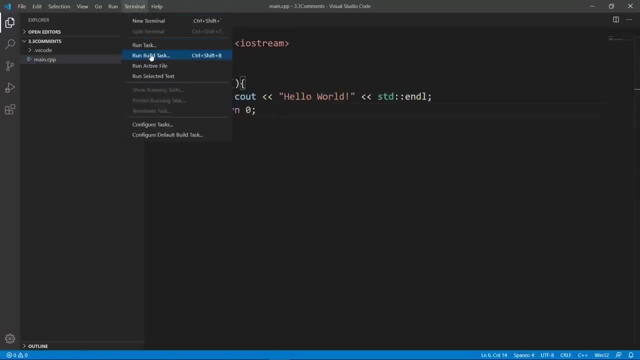 So make sure your code looks like this. Try to build it To make sure it is working fine. This is going to run the gcc task build. We can click on the terminal here And it is going to close the terminal And we can open a new terminal here. 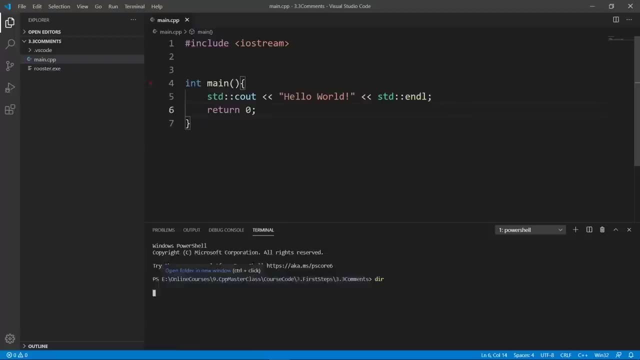 If we want, If we do, dir, We are going to find our rooster program inside, We can run it And it is going to say: hello world. We already know how to do this from the last lecture And in this one. 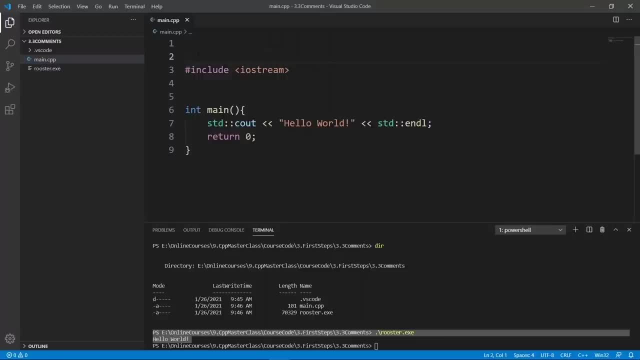 We are going to say: stdc out comments. The first thing you can do Is use slash slash. So let's do that And let's put some message here. This brings And the iostream library. This is a nice message. 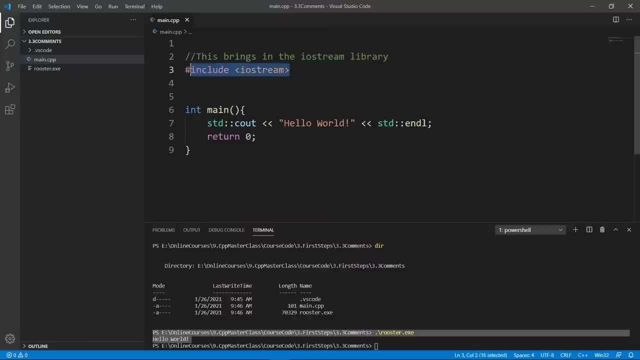 That is going to give some more information About this statement To whoever might be reading this program. And this is called a one line comment. You can really put this wherever you want In your C++ file. We can go in the main function, for example: 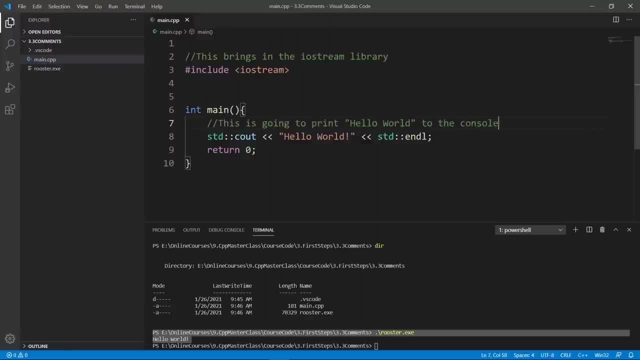 And we are going to print hello world To the console or the terminal. We can really put this anywhere. We can even put it after the return statement here And really put in Whatever piece of information we think Is going to make sense. 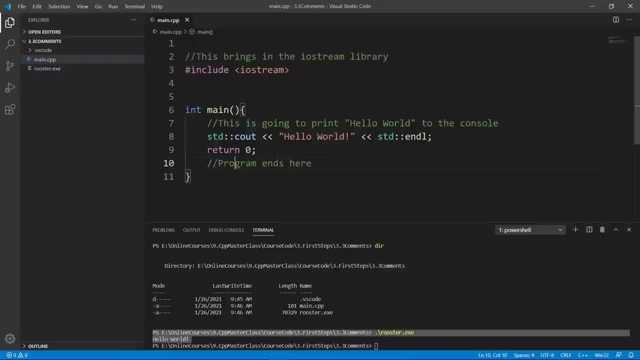 To whoever is going to be reading our program. Okay, This is how you do a one line comment. You can also do comments Across different lines And the way you do that, You put that in the slash star And go down. 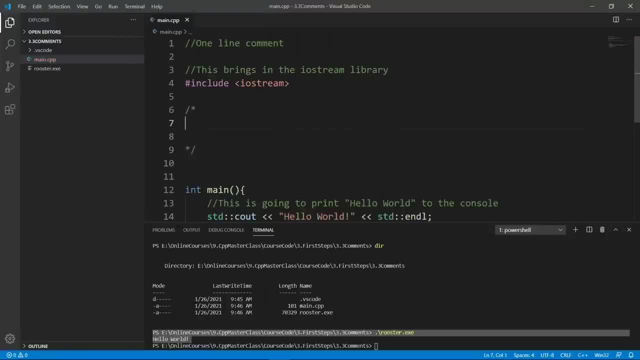 And say star slash, like this, And whatever is going to be in the middle. here Is going to be a comment. This is usually called a block comment. You can put in whatever you want, So if you have a piece of text That you would like to use as a comment, 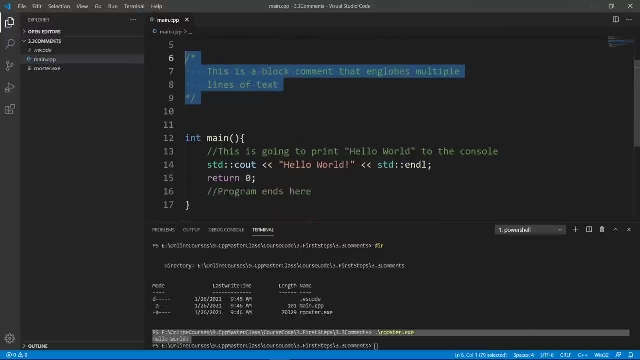 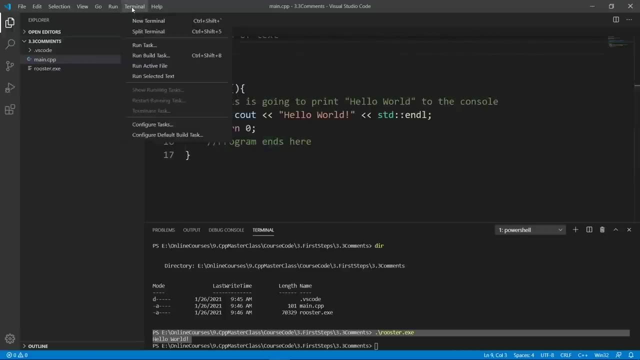 In your program. This is one way you can do this. One thing you should know, though, Is that you cannot nest these things, But before we do that, Let's try to build our program To really show that there is no problem. 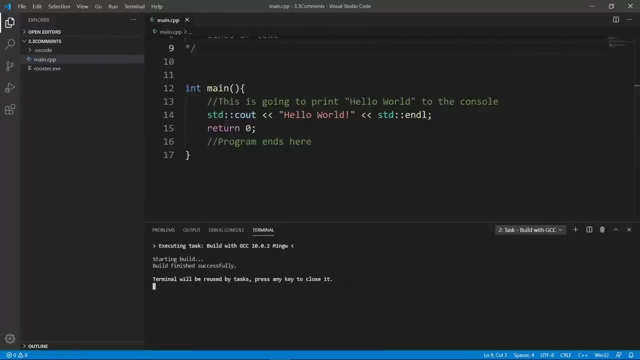 If we have these comments in And if we click on this terminal And hit enter And hit clear To clear things out in the terminal, We can try to run our rooster program And it's going to say: hello world. You see that, all these green lines, 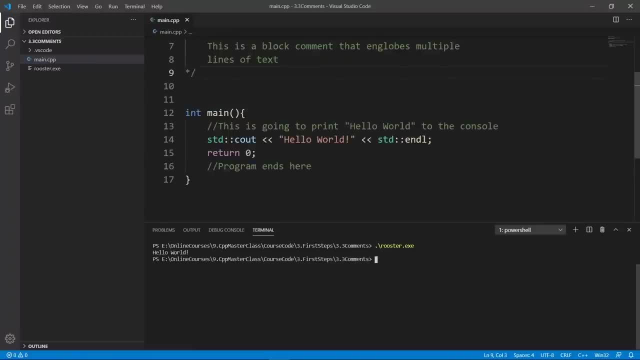 Which are comments, Are really not affecting the program. All the compiler is going to care about Is this include thing. It's going to care about the main function here. It's going to ignore these green things. It's going to be like these green lines. 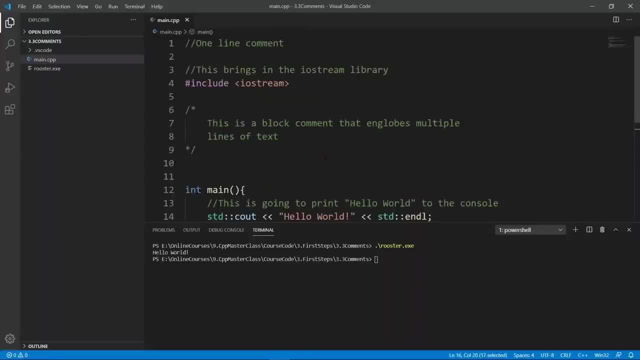 That are our comments That are not in there. This is the effect comments have on your program, And we're going to be using this a lot in this course. One thing you should know, though, Is that you cannot nest These block comments. 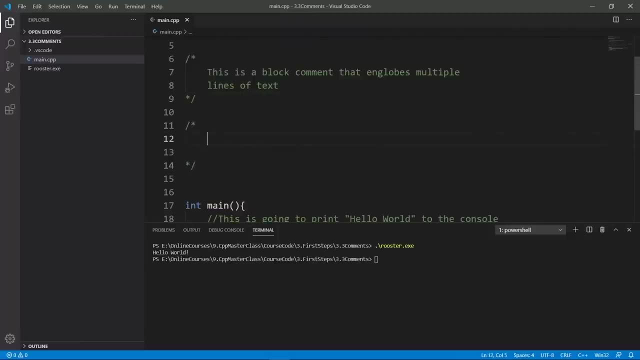 So if you try to do something like this And say this is one comment And come again And say this is another comment, You see that we have problems already. Nesting is not allowed. You're going to get a compiler error. 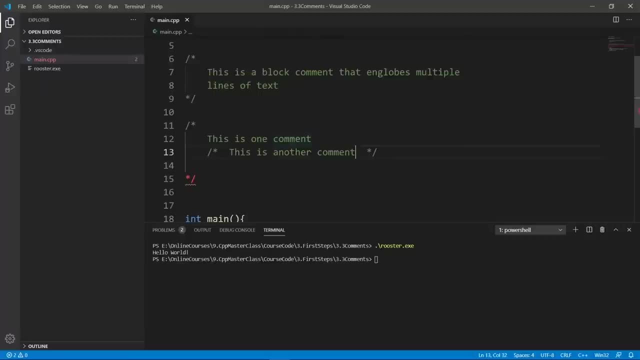 And we're going to learn more about these errors In the next lecture. So just don't nest these block comments. If you do that, You're going to get some confusing errors And this is going to be the cause for them. So don't nest your block comments. 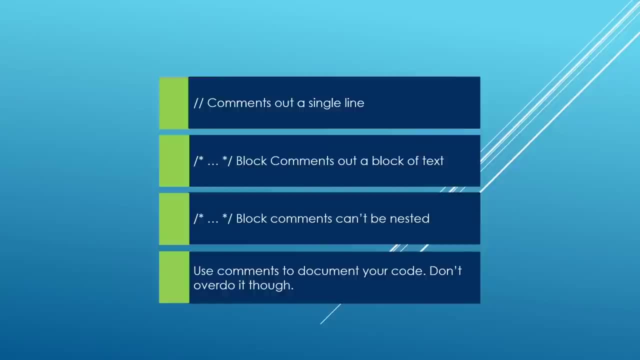 It's going to give you headaches. Okay, This is really all we set out to do in this lecture. Learning about comments in C++. You can do one line comments On a single line like this: You can do block comments To comment out a block of text. 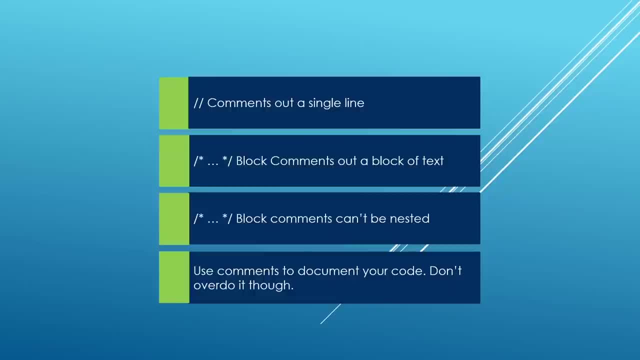 You can't nest your block comments Because that's going to give you a lot of problems. You don't want that And really use comments wisely And don't overdo it, Because it's going to turn your program into a novel. 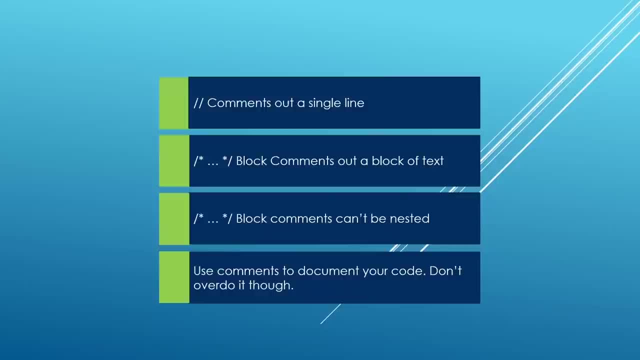 And I don't think people want that. So use this feature when you need it To give some more information about your code, And don't overdo this. We are going to stop here in this lecture. In the next one We're going to learn about different kinds of errors. 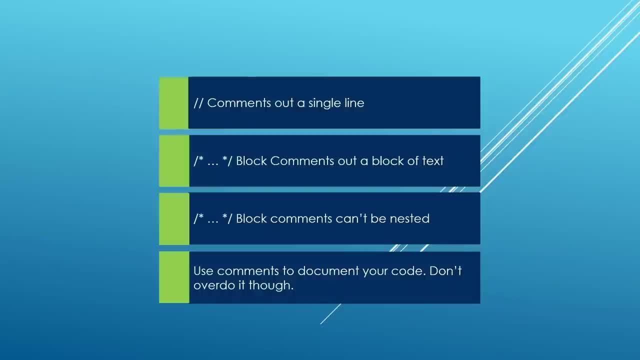 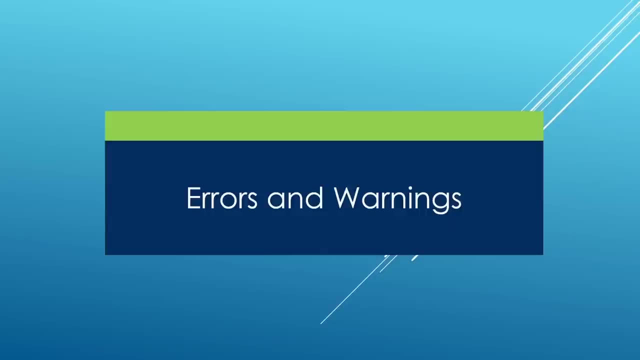 And warnings You can see in your C++ program. Go ahead and finish up here And meet me there. In this lecture We're going to learn about errors and warnings In your C++ programs. There are three kinds of errors. 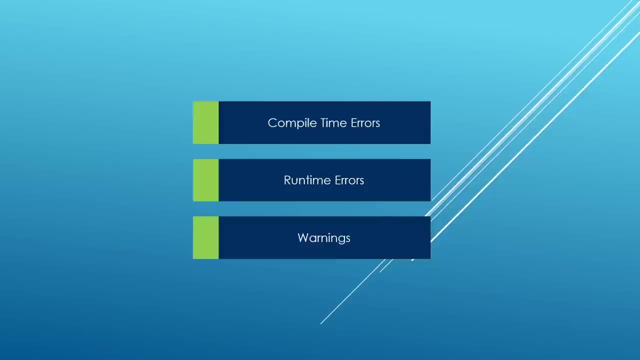 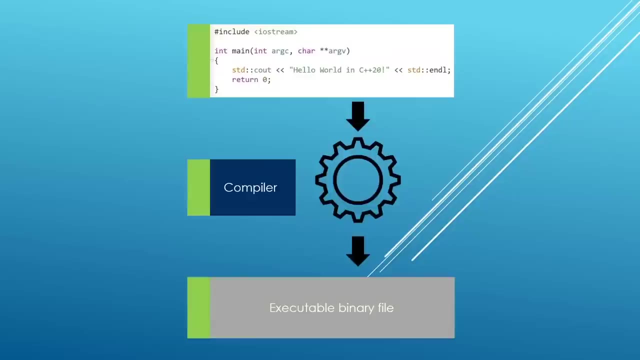 Or warnings you can get. You can get compile time errors, You can get runtime errors And you can get warnings. But what is really meant by these things? Remember the ultimate goal Of every developer, Or every C++ developer, In our case, here. 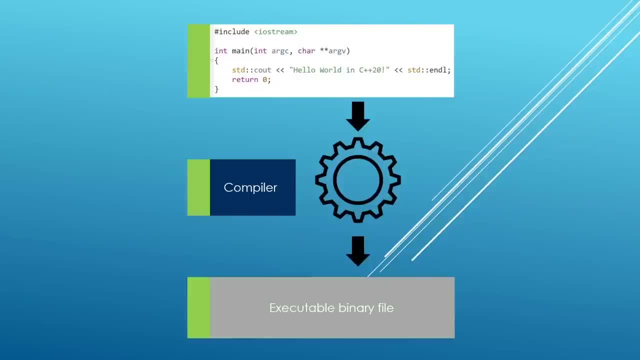 Is to be able to generate Every executable file From the C++ code, And we have to run the code through the compiler To be able to do that, And one thing you should know Is that there is a set of requirements. 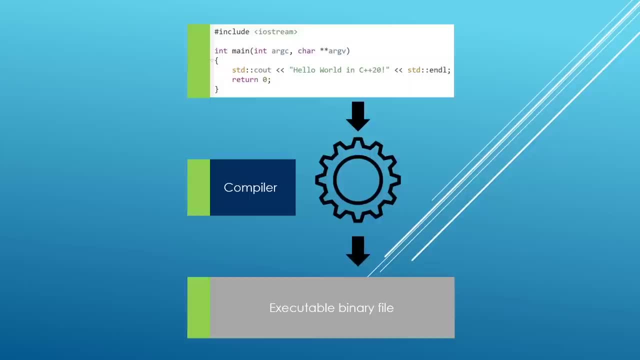 That the compiler enforces On our code For it to be able to compile successfully. And those requirements are the rules, really, That we have to follow In our C++ program, And if we break those rules We're going to get problems. 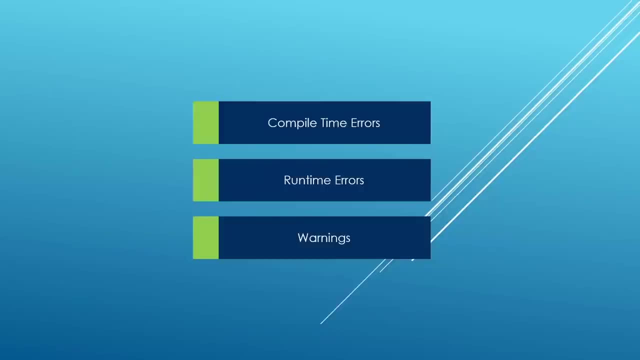 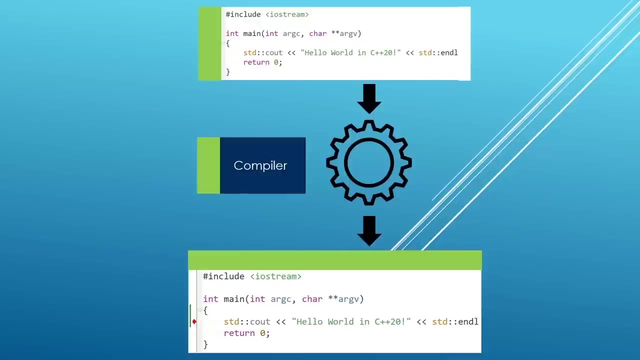 Of compile time errors, Runtime errors or warnings. Let's look at Compile time errors in detail. Here we have a simple C++ program That has a few problems. We have forgotten To put the semicolon at the end Of our stdcout. 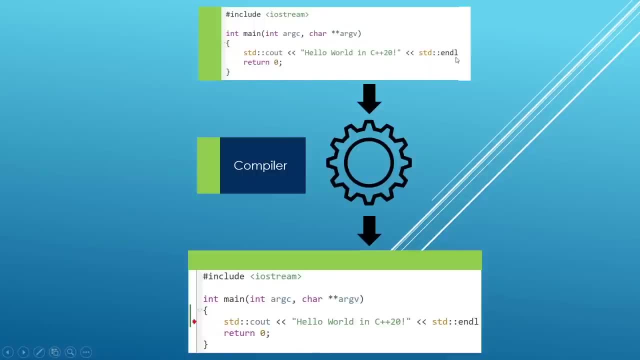 Statement here And the compiler is going to freak out Because of this. If we compile this program, We're going to get a bunch of errors And the IDE is going to show us this problem. The IDE is going to give you different errors. 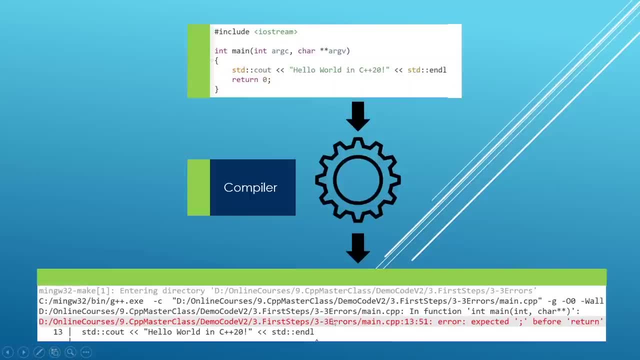 For example, here I was using code light And it was saying: Error: expected semicolon before return Or something like this. So this is a compiler error And if you have this kind of errors, Your program is not going to compile. 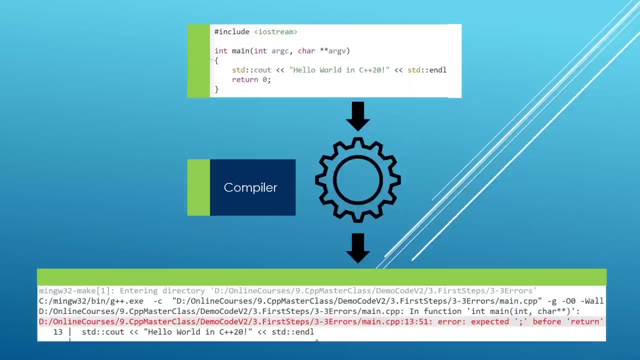 Compilation is going to fail, You're going to get this error And you're not going to get your binary executable, And when you have this, You basically have to go back and fix this problem, Compile again. This is what a compile time error is. 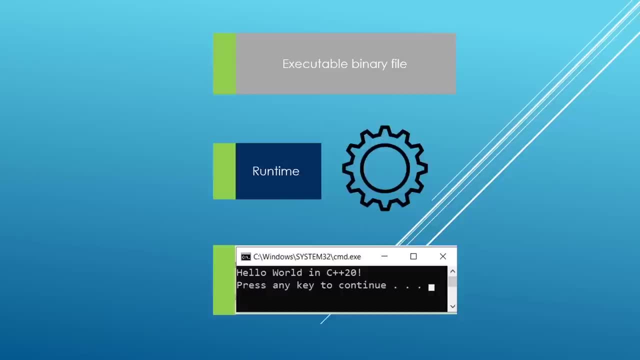 Another thing you can have Is the run time error. This is not going to cause a compile time error. The compilation is going to succeed, But when you run the program, It's not going to do what you intended it To do in the first place. 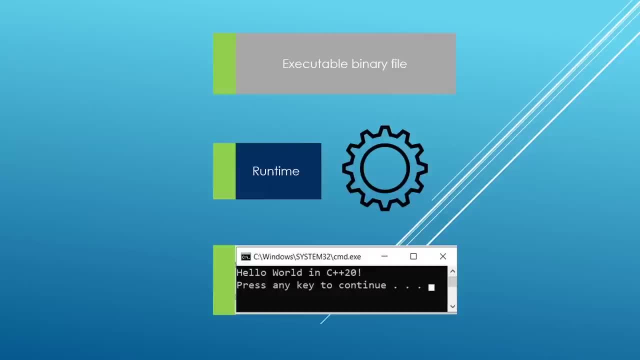 For example, You may want it to print green On some user interface. It's going to print gray Or whatever. It's really not going to do what you want. So it's a logical error And you have to fix it. 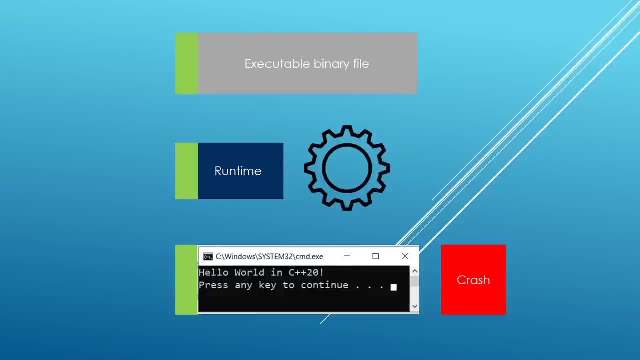 To get rid of this. And another thing you should know Is that sometimes these run time errors Can cause your program To fail and terminate immediately, And we say that the program has crashed. We're going to see an example of this. 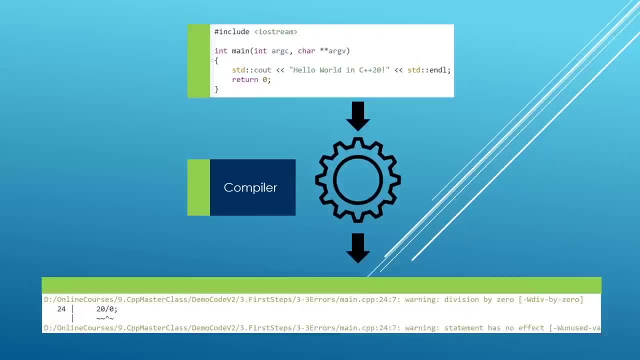 In a minute. The last kind of problem you can have in your program Is a warning. This is a problem that is not Serious enough for the compiler To halt your compilation. Compilation is going to succeed, But this is basically The compiler telling you. 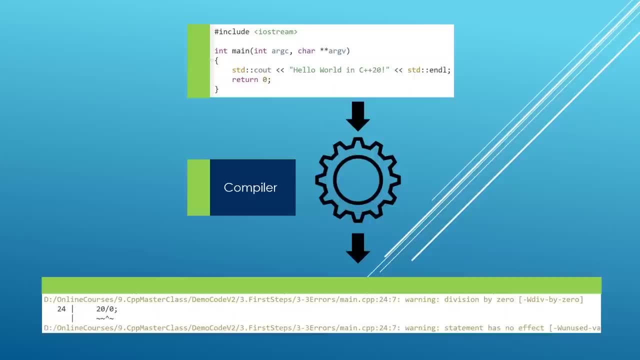 You are doing something that has some problems And you should really fix it Before it becomes a serious problem. So that's going to be a warning. For example, here you see, Some compilers can warn you When you divide stuff by zero. 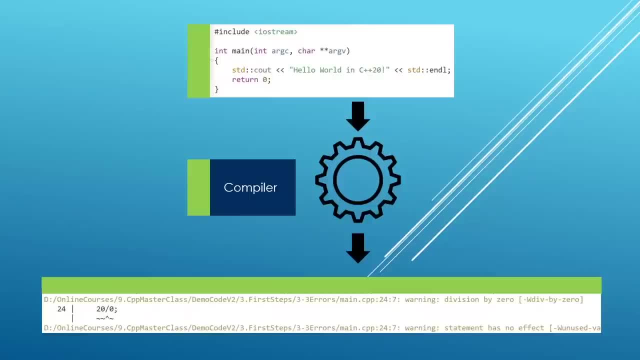 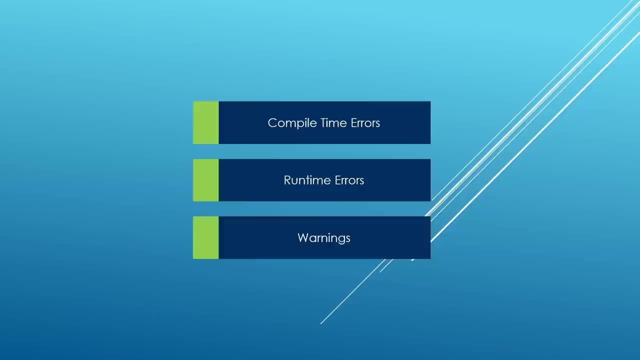 And we're going to see how this works. The main message in this lecture Is that you may have problems in your program, And they are going to come in three forms. Some are going to be compile time errors, Some are going to be 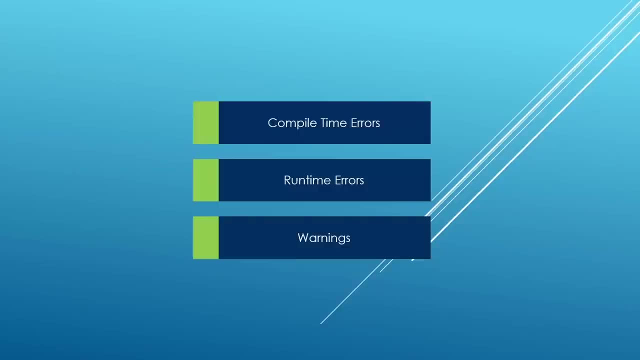 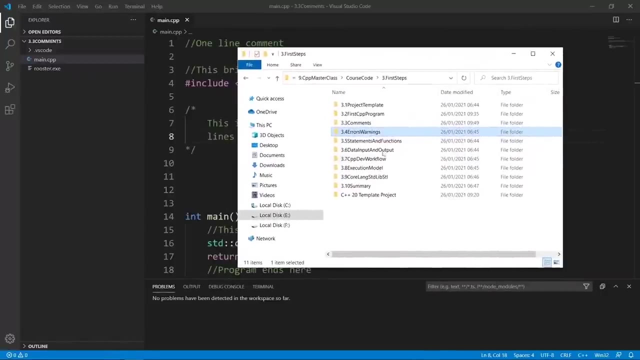 Warnings: We are going to hop over to Visual studio code And actually play with this. Okay, here I am in visual studio code. The first thing I'm going to do Is to set up The template project we're going to be using. 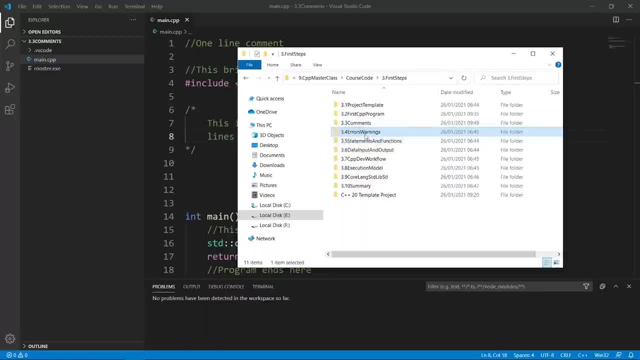 In our project here. The project is going to leave in this folder Errors and warnings. I am going to copy over the files And I am going to go in the current project We're going to be working on And I am going to open this folder. 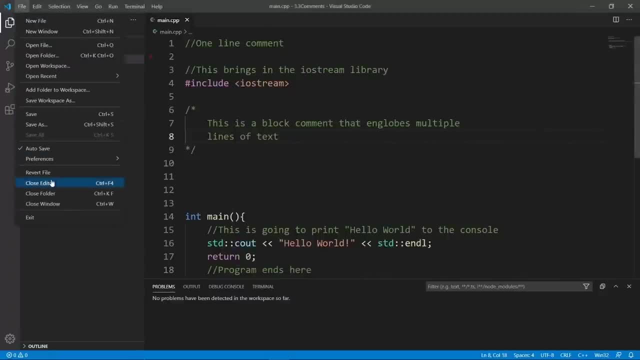 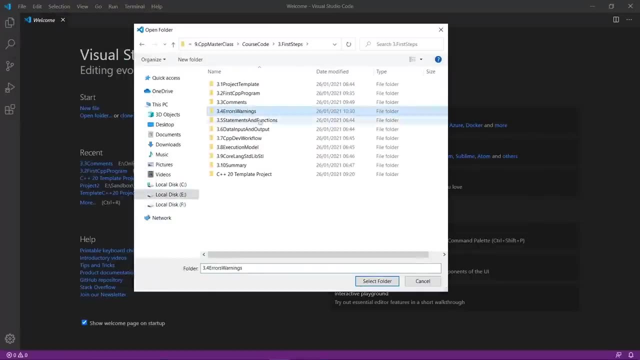 In visual studio code. I am going to go to file- Close folder. I am going to close this one And I am going to open our new project. I am going to browse to it. The project is this one. I am going to select it. 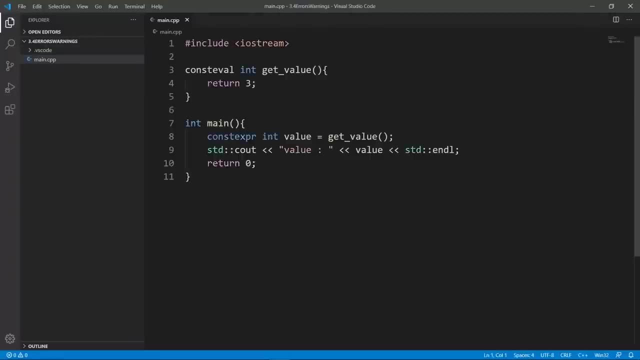 And select folder And it is going to open up In visual studio code. I am going to close this welcome screen And open our main CPP file. We're going to get rid of this const eval thing. We're going to get there in due time. 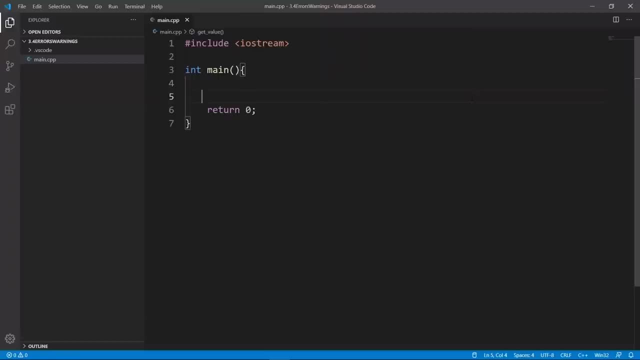 What we want to see is Compile time errors. We're going to put in our stdc out statement Hello world, As we usually do. We're going to end this Stdendl And we're going to remove The semicolon on purpose. 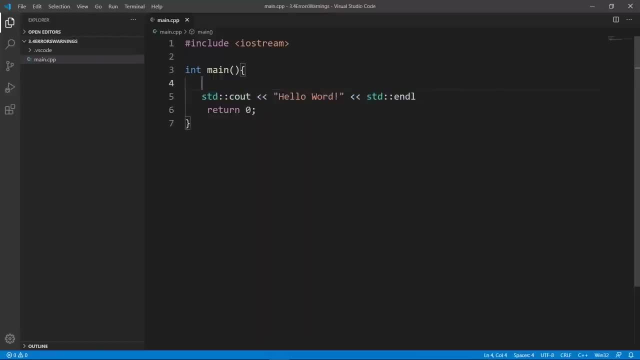 And if we try to compile our program like this, We're going to get a compile time error. This is what we want to see. So let's try and build our program. We're going to run the task To build with gcc. 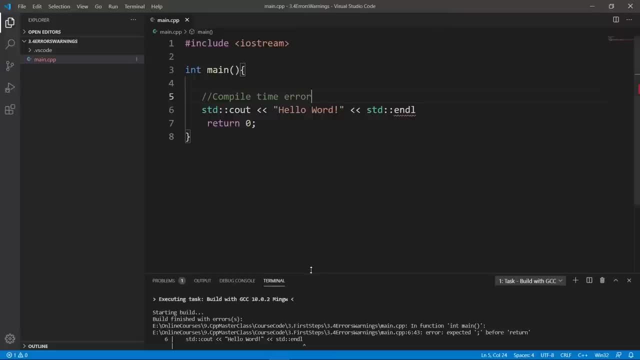 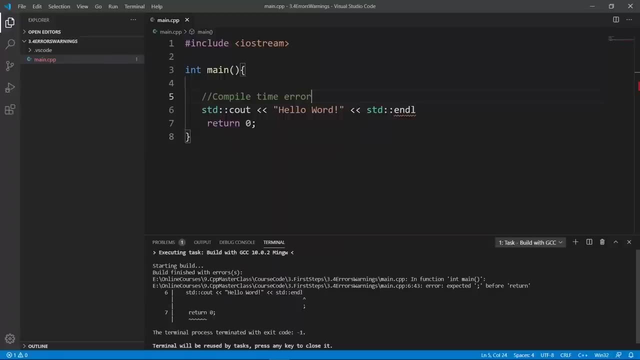 And you see that the build fails. We're going to get a bunch of errors In our terminal. It's going to say in function int main Expected a semicolon before return. It's going to try its best To tell you what the problem is. 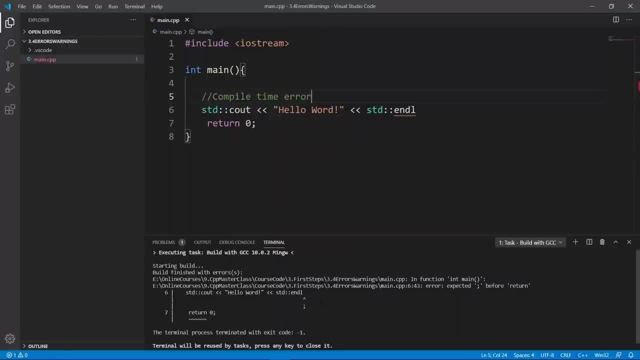 But sometimes these errors Can be really confusing. In this case it is really easy, Because we introduced this error on purpose. So we're going to fix it in a minute, But before we do that, I want you to see these problems. 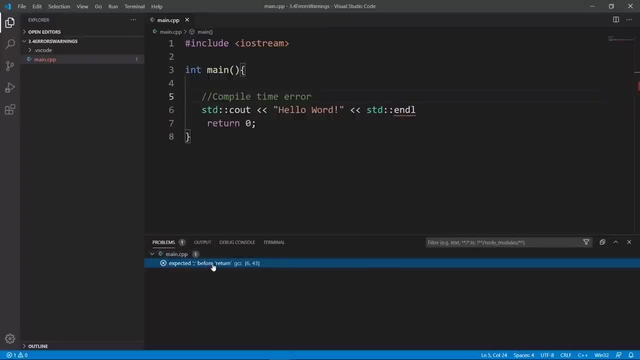 In the problems tab. It is where the problems are going to show up In visual studio code, So you should see your problems In here or through the terminal here. Okay, one thing you should know Is that when you have a compiler error, 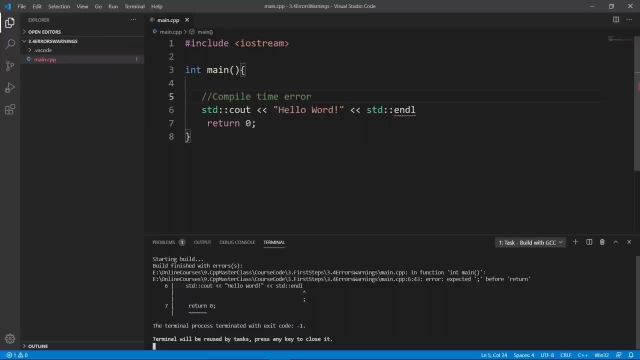 Compilation is not going to succeed And you're not going to have your binary file, Which is what you really want. So, to fix this problem, We're going to put in our semicolon here, We're going to build again, We're going to go to terminal. 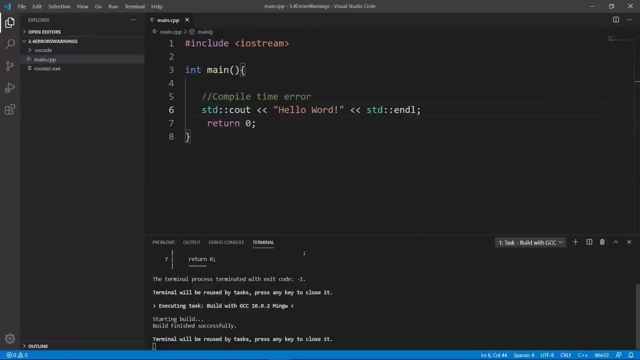 Run task And we can see that compilation Is going to succeed And we have our program here. We can run it through the terminal here. So we're going to click. The terminal is going to go away, But we can open our own. 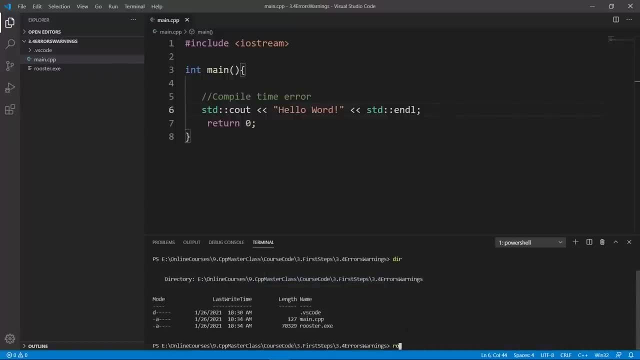 And if we do there We're going to see our files in here And we can run our program. We can say rooster And if we run We're going to have hello world. So I hope this really makes it very clear. 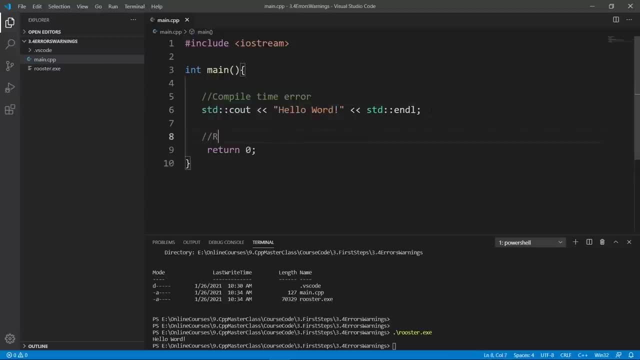 The other one is a runtime error, And this comes in the form of Things that don't work, As you really expected. So let's say we are trying to Do some computation in our program. We try to Take 7.. 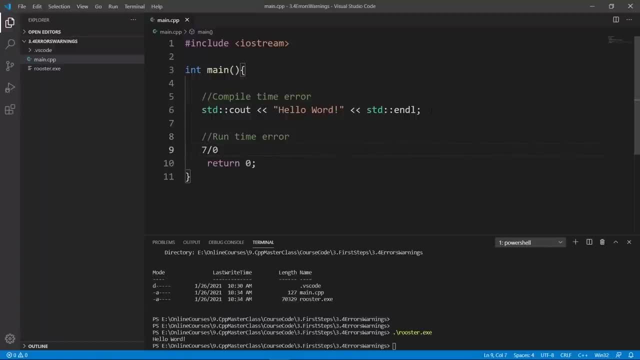 And divide this by 0.. For example- And this is a statement that is allowed in C++. So let's try and build this And see what we get, Because this is a common Scenario where we have Runtime errors. We're going to run the task. 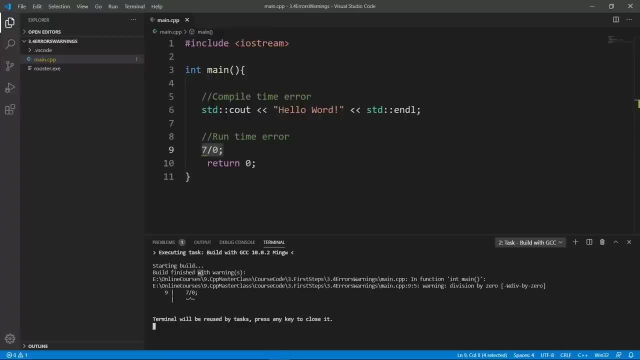 To build with gcc. Okay, if we do this, You see that build finished with warnings, We didn't get a compile time error And our build was successful. So to really prove this, I'm going to go back in our directory. I'm going to do dir. 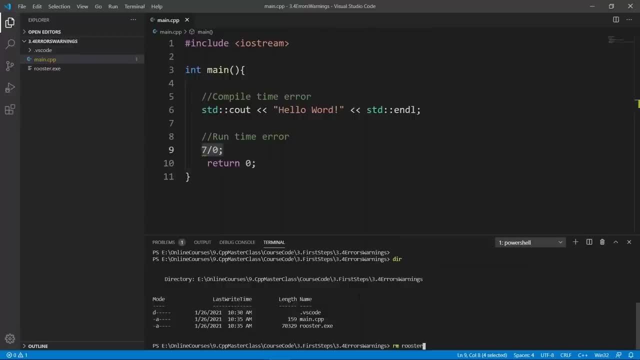 You're going to see that rooster is there. I'm going to remove it. I'm going to say roosterexe. This is how we remove stuff From the command line. Again, The executable file should be gone. So let's try and build with this statement in: 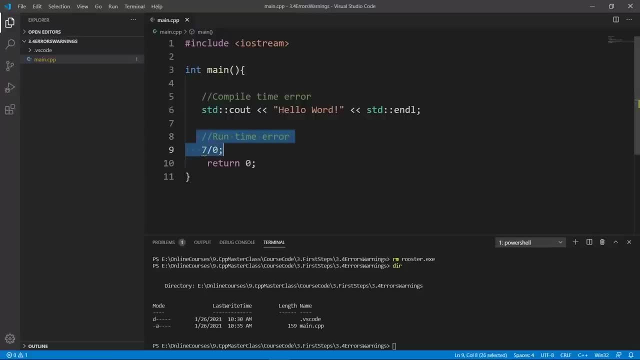 And you're going to see that we get a warning And not a compile time error Like we had here. So we're going to go to terminal Run task, We're going to build with gcc And you're going to see that we're going to have our executable here. 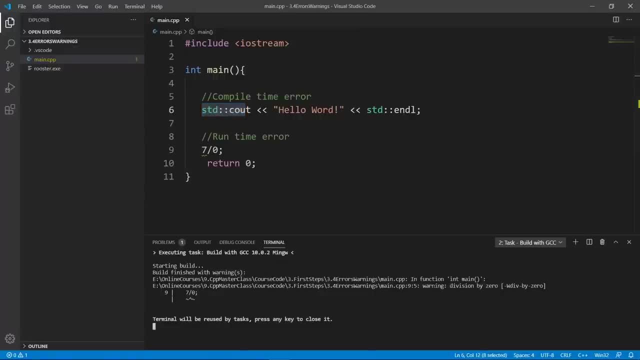 But we had a warning And it's saying that division by 0. Was detected in our program And it is a recipe for disaster. So why is it a disaster? Let's try and run this program, So we're going to dir. 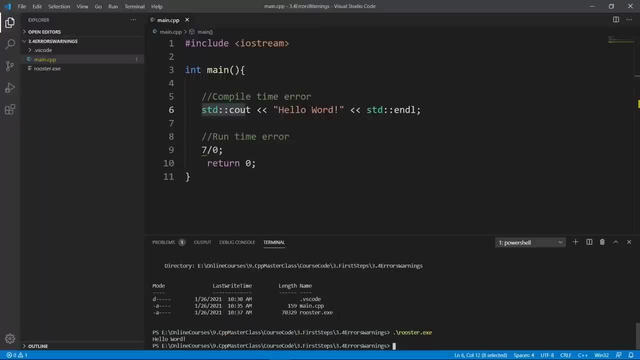 To prove. it's here And we're going to run it. If we run it It's going to say hello world And it's going to end. Let's try and actually use our own terminal To see if we have a better chance of seeing the problem here. 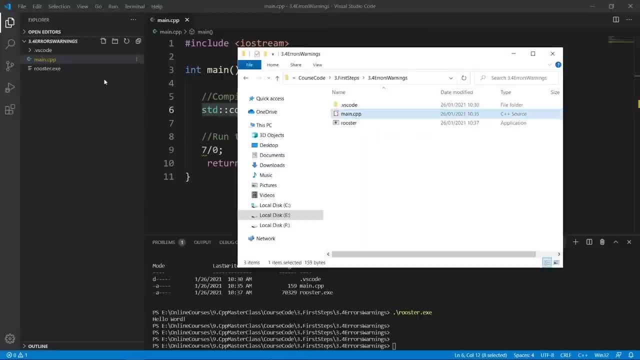 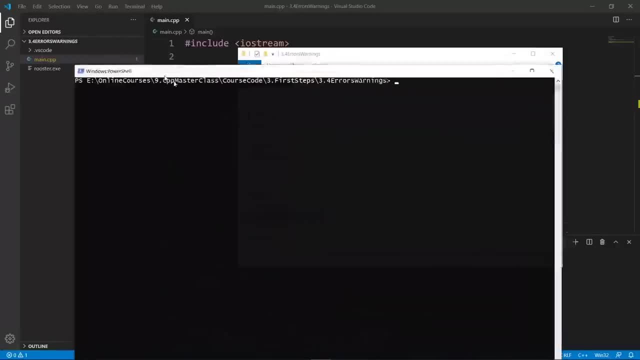 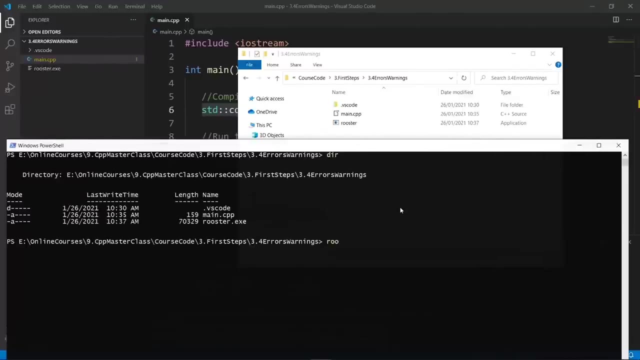 So I'm going to reveal in explorer By clicking on main cpp, And I'm going to try and open a terminal Window here- Power shell- That we open ourselves And it's going to be new to you By now, So we're going to do dir in here. 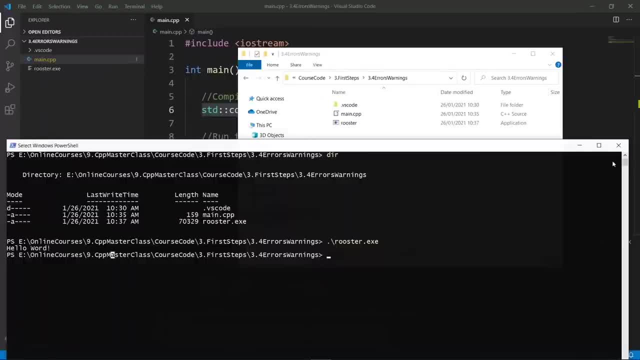 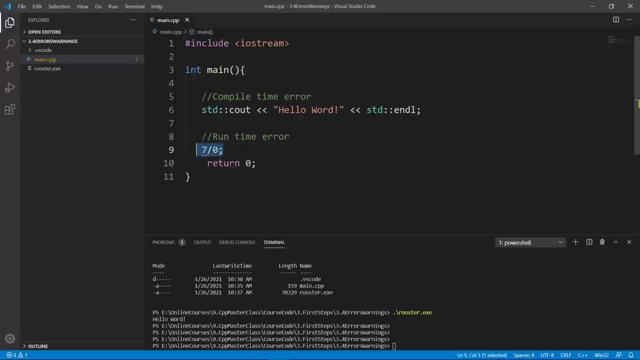 And we're going to try and run the program And it's going to run, So it's not really giving us a run time Error here Because we're not capturing this Or trying to use the result of this division here We're just doing the division. 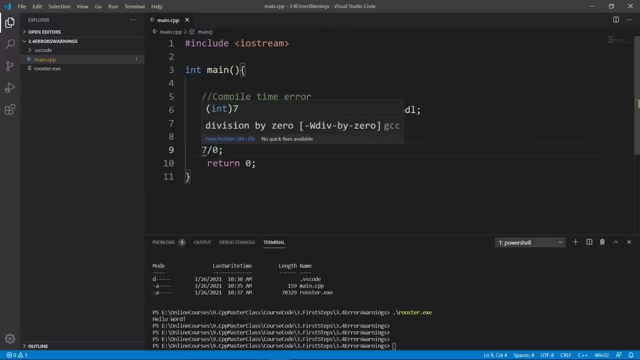 Which is a problem. So let's try and capture this. We haven't learned about variables yet, But what we're going to do now Is do int value The result of this division To this value, And let's try printing the result. 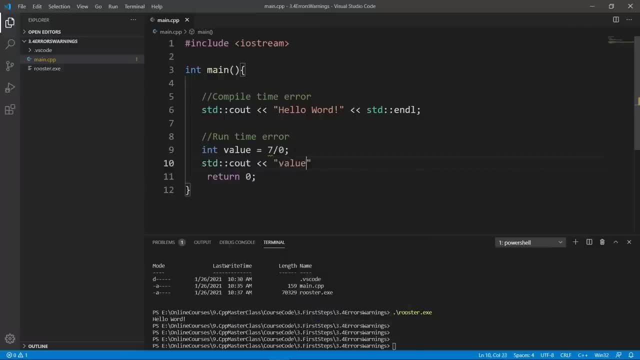 Of dividing a number by zero. So we're going to do stdcout And we're going to say value, And this is how you can print a value out On the console. Okay, now that we have this end, Let's try and build. 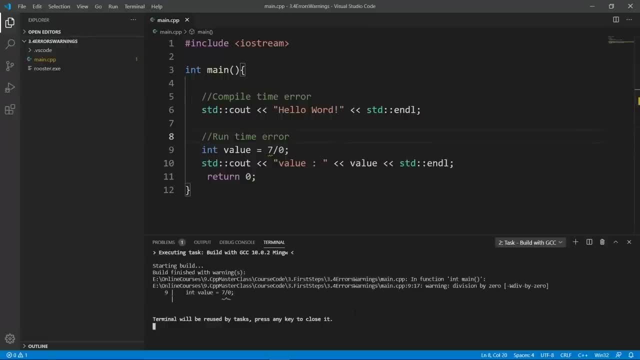 We're going to run task and build with gcc, We're going to get the same warning. But if we try to run the program, We're not going to get what we expect. We expect it to say hello world And print the value. 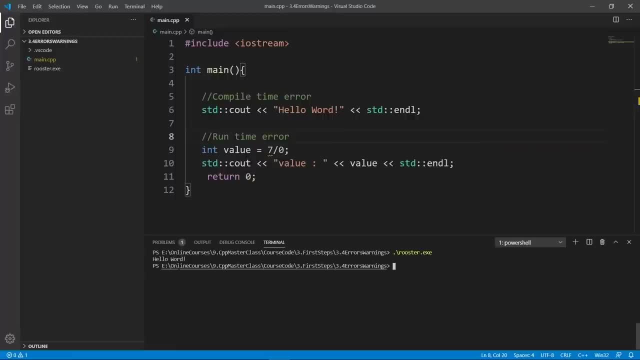 But you see that it's really struggling to print the value And it gave up And ended immediately. So this is one example of a runtime error That you can face in your program. There are many other kinds That we're going to see as we progress in the course. 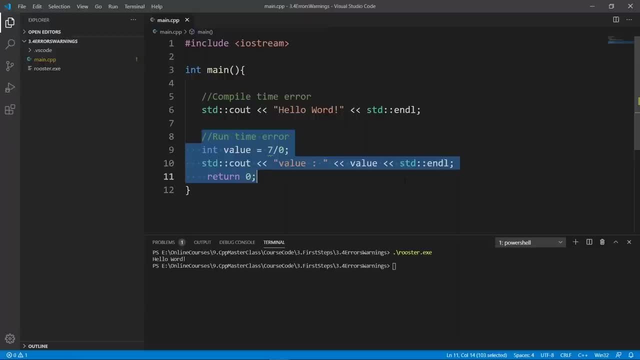 Here. we are just trying to raise your awareness On these problems So that you can know how to fix them When they come up. Okay, so this is all I can share with you now About runtime errors. We also had a chance to see that. 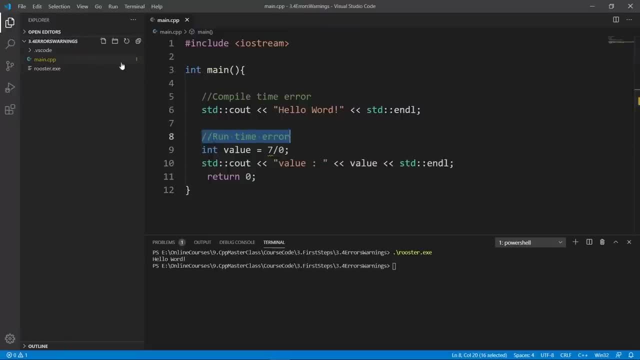 This is also going to give you a warning, And a visual studio code here Is also helping out, Telling us that we may have a problem. It's turning the main cpp file yellow And it's saying that there is one problem. 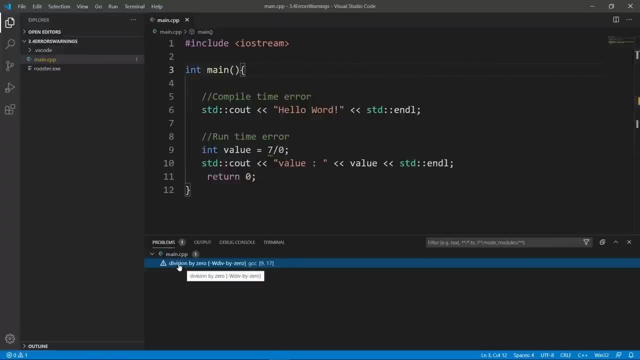 In this file And if you go here, You're going to see that we have a warning here. Okay, so this is one way you have to see this. So this is not recommended to do, So we're going to comment this out. 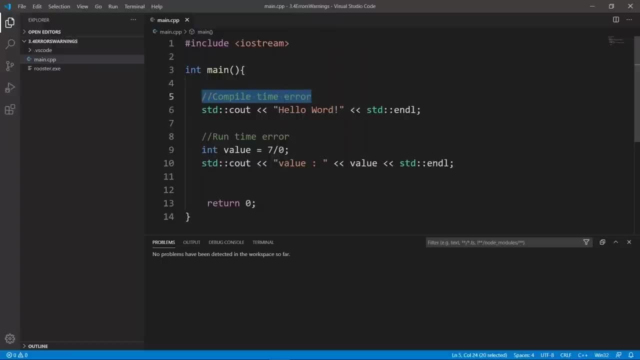 Okay, this is really all I had to share in this lecture. We had a chance to look at compile time Errors. We also had a chance to look at warnings And runtime errors. using this example: If you get a warning, It is a message the compiler is giving you. 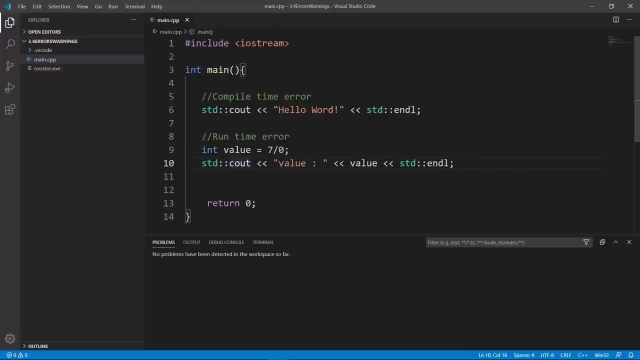 That you should really look it up And fix the problem Before it becomes more serious. Compile time errors are going to cause Your compilation to fail, And that's a really good thing, Because the compiler is going to stop you From generating a binary. 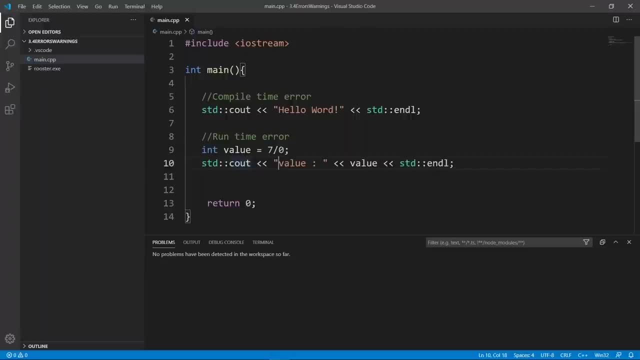 That doesn't really do what you expect it to do, So that's a good thing. Sometimes the compiler won't give you A compile error And you have a chance to run into a runtime error And that's really bad. So be careful about these things. 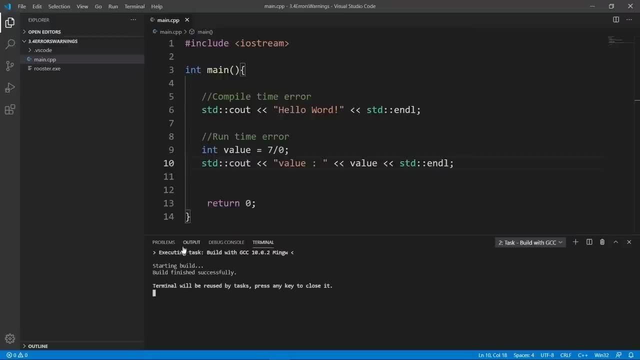 And when you have problems, Visual Studio Code is going to show you The problem in terminal Or in this problems tab And you're going to be able to fix it up. We're going to stop here in this lecture. In the next one we're going to learn a little more. 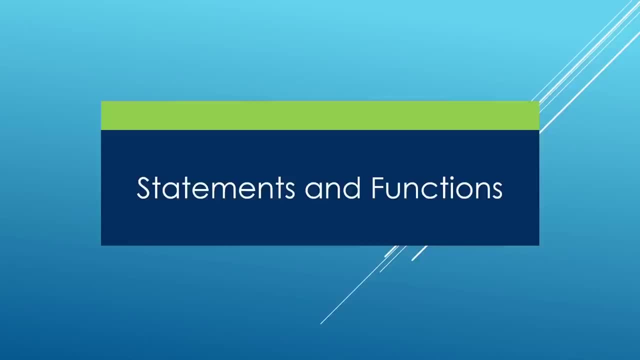 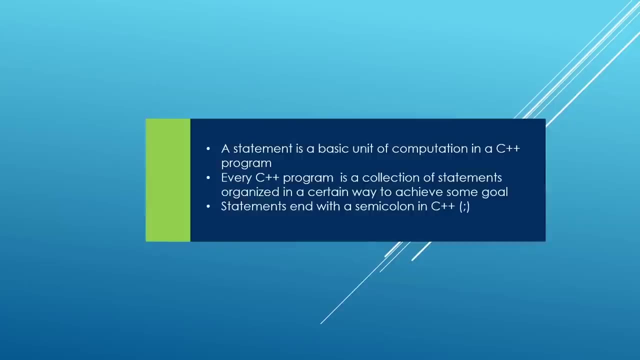 About statements and functions. Go ahead and finish up here And meet me there. In the next lecture We'll talk about statements and functions In C++. A statement is a basic unit of computation In C++. You can say that it is the smallest thing. 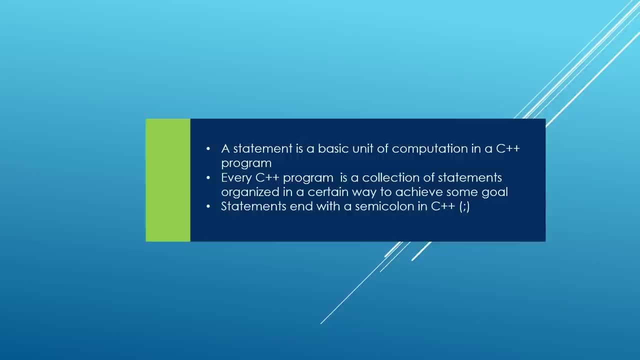 Your CPU can execute in your program. Every C++ program Is a collection of statements, So you're going to have a bunch of statements That are organized in a certain way To achieve whatever it is you want, And statements in C++. 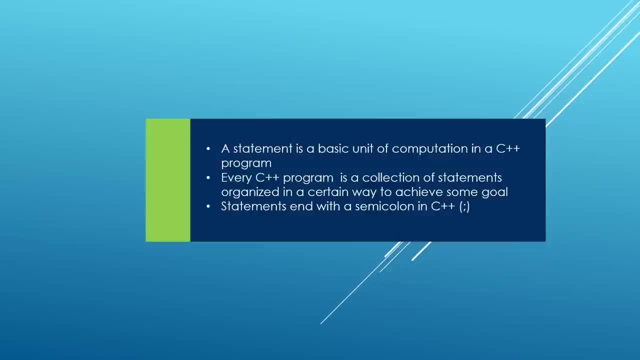 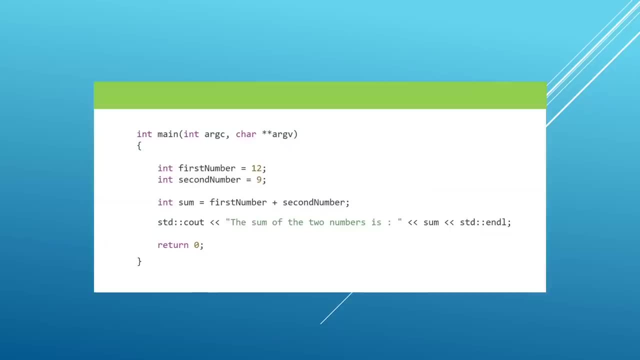 Must end with a semicolon. We saw in the last lecture That not putting that semicolon Is going to result in a compile time error. Here is a basic sample C++ program That we're going to use To learn about statements. 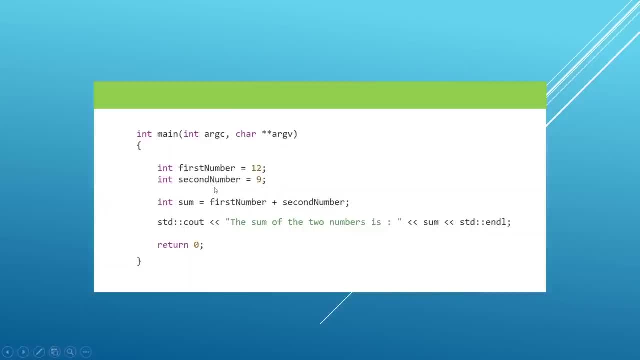 In the main function. here We have two variables declared. We haven't really learned about variables, But they are a way to store data In your program. And here we are storing two decimal numbers. One is called first number, The second is called second number. 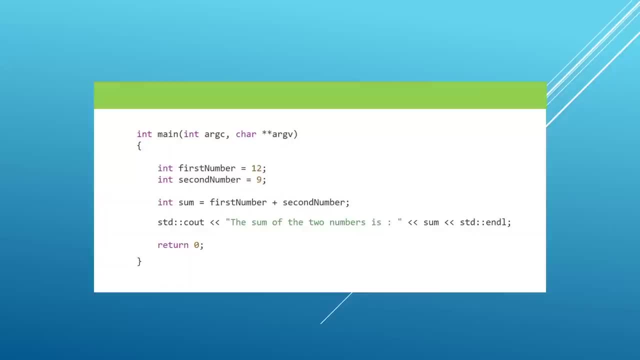 We can do something With these variables That we have in our program. For example, we can add them To have another variable in our program And we can print that. So you see, here We are saying stdcout, The sum of two numbers is sum. 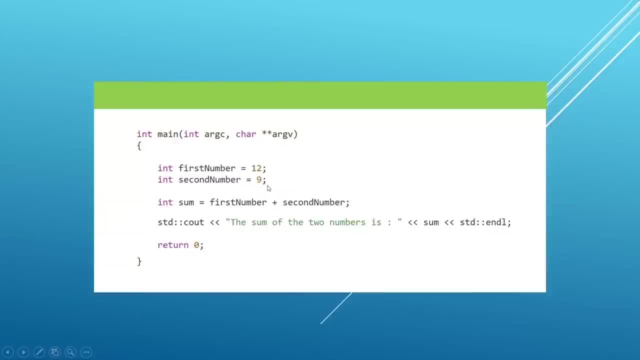 So this is going to print 21. Because it's going to add 12 and 9.. And the result of that Is going to be displayed on the terminal If we run this program. What I really want you to notice Is a statement in C++. 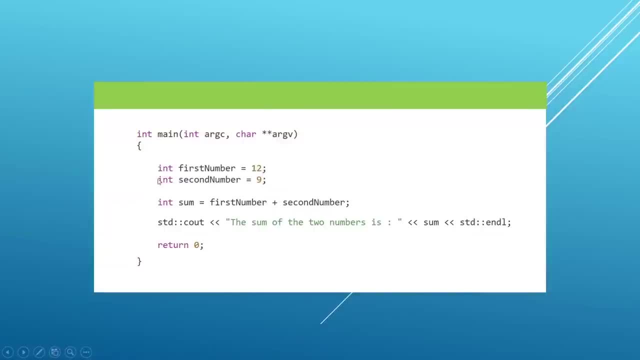 So it must end with a semicolon. The line here with second number Is also a statement, So it must end with a semicolon. Every single line we have here In the main function Is really a statement And it must end with a semicolon. 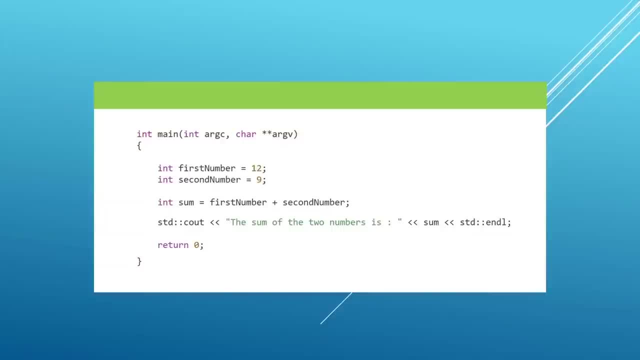 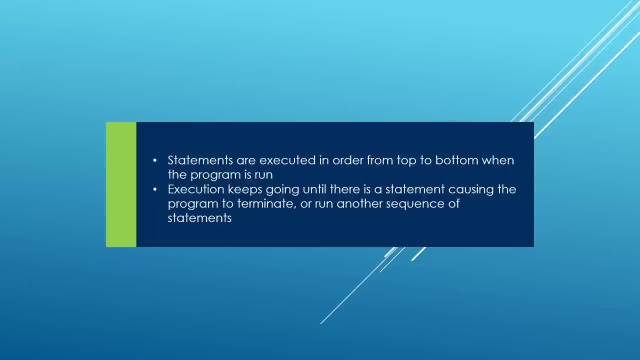 If we don't put the semicolon in place, We're going to get a compiler error. Okay, one other thing That is really important To keep in mind Is that statements are executed By the program And the order is from top to bottom. 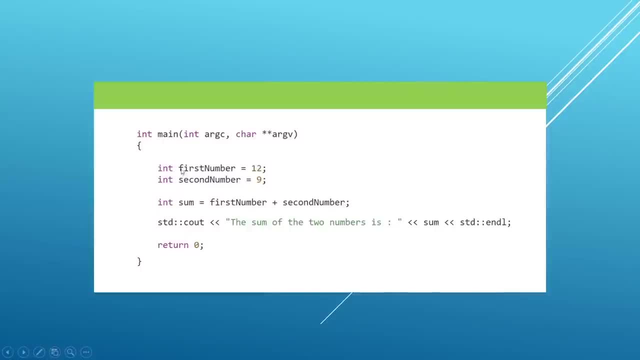 If we go back to our program here. So the first statement Is the one with first number here. 12 is going to be stalled in memory When this statement is executed By your computer And we're going to go to the second statement. 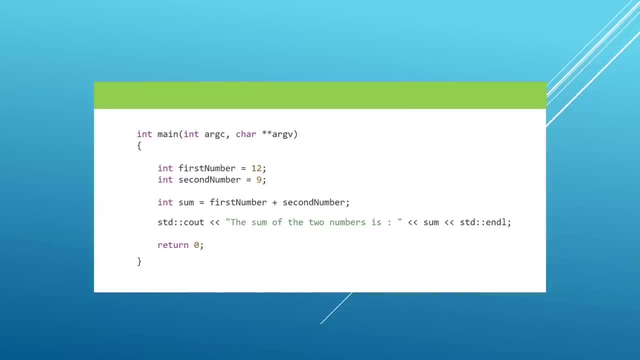 With second number And we're going to keep going Until we hit the end of the main function And the return statement is going to execute And when the main function returns Or terminates, The return value sent to your operating system And it's going to know. 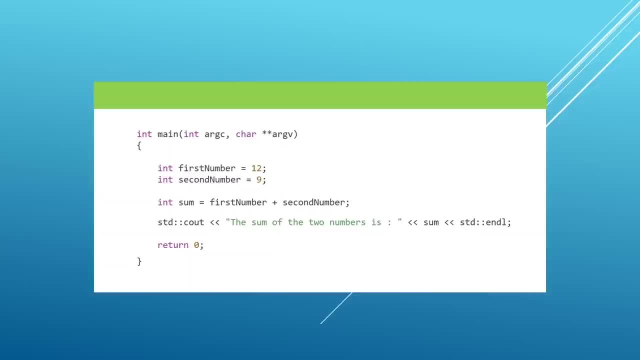 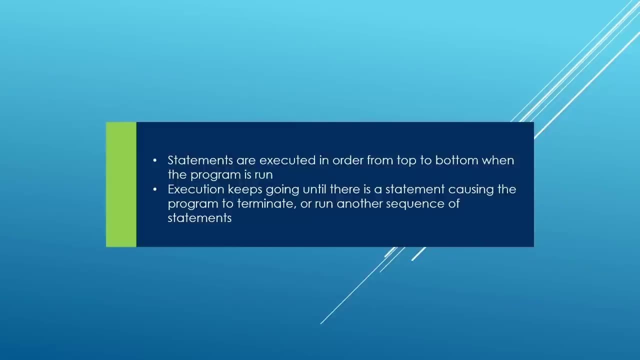 If your program ended successfully Or with a problem And the operating system is going to know What to do with that information. Execution keeps going Until we hit the end of the program Or if there is any other condition Causing for the program to terminate. 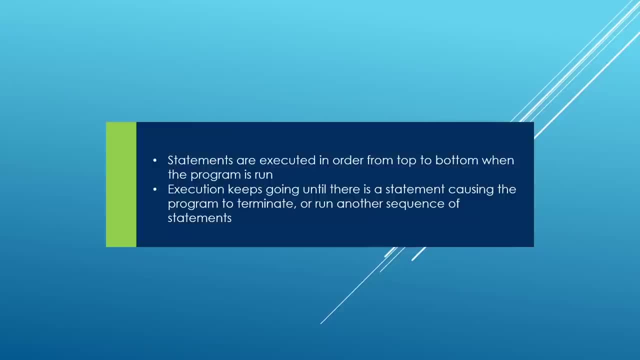 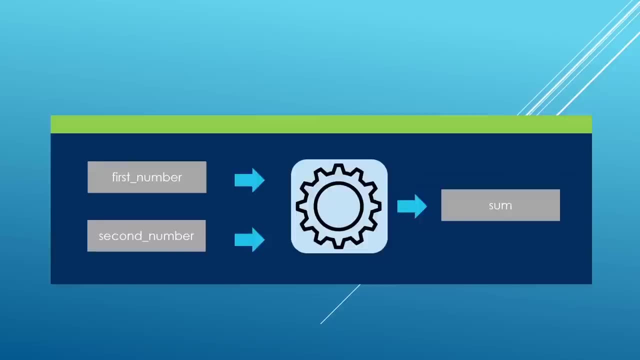 And we're going to have more details About these things later. I just want you to know That the statements are executed in order In your main function And we're going to have a look at The concept of functions. A function is really like a machine. 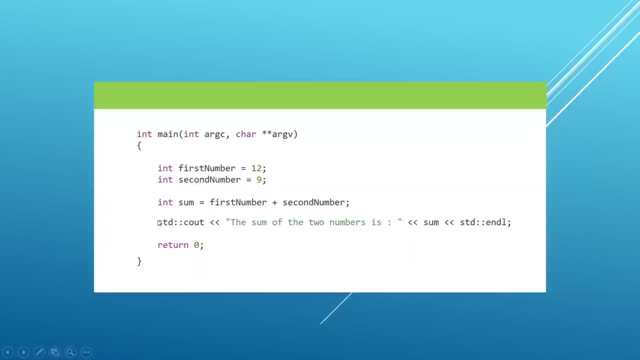 You give it input And it's going to give you output. If we look at the operation Here to add first number to second number, We can consider first number And second number As input to the function And sum is the output of the function. 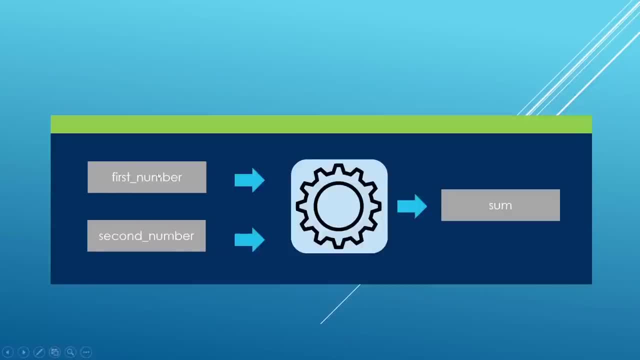 We can visualize that like this: So we have a first number And a second number And we're going to get the result Of this function In a return value Or something that we get out of the function As our result. 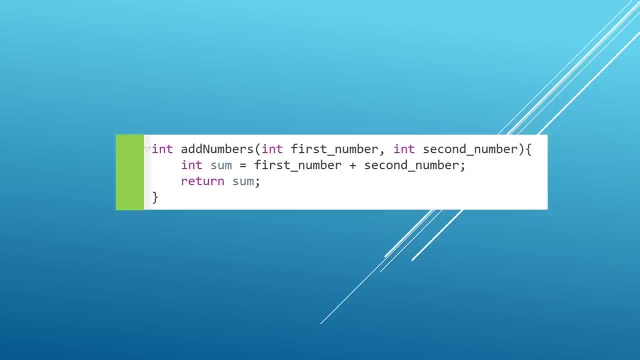 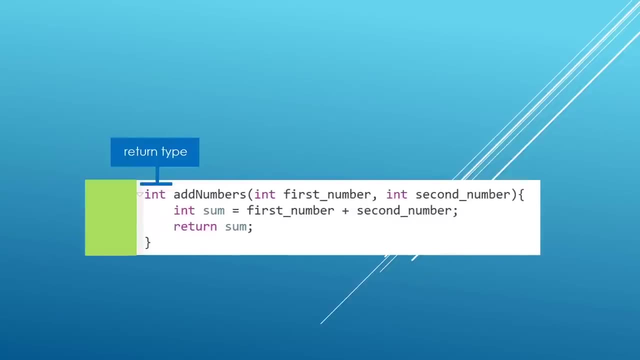 C++ has a special syntax We use to define functions. This is our function: to add numbers. On the left we have an integer Which is code name For a whole number in C++. It's a number without decimal points And it's a whole number. 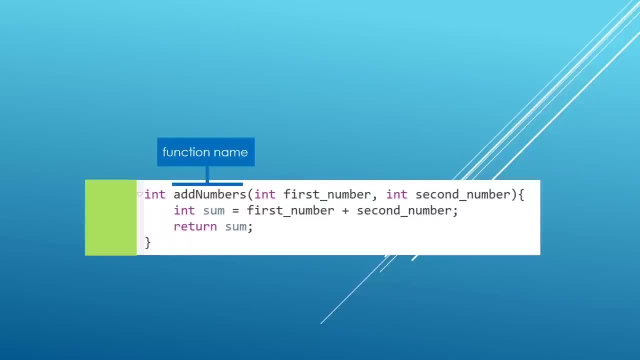 After that we have the name of the function And we can name it whatever we want, And after that We're going to have the list of parameters That we can pass to the function, And this is going to work as the input to the function. 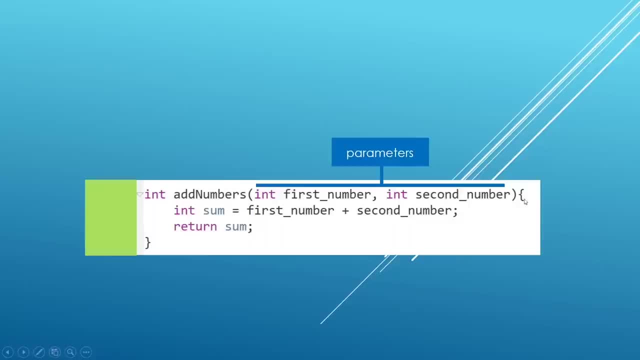 After you do that, You're going to have a pair of curly braces. The one is here, The other is here to the end, And within those curly braces It's going to be the body of the function Inside the function. You see that we are declaring a variable. 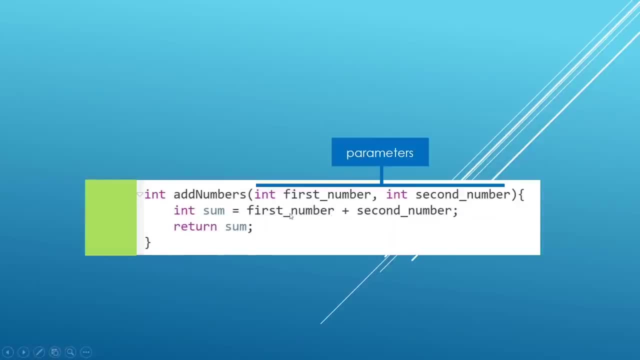 Which is called sum, And we are storing the sum of first number And second number And we are making this function Return the sum as the result And we're going to be able to capture it If we call this function In a function like main. 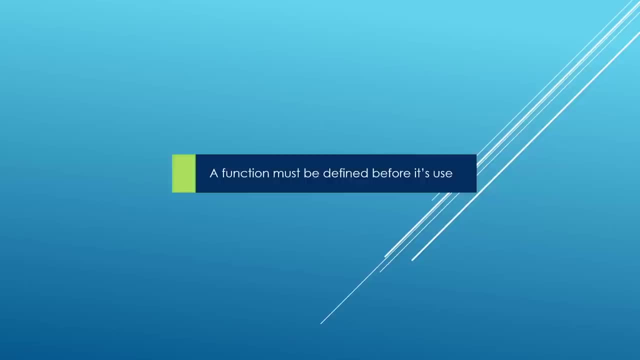 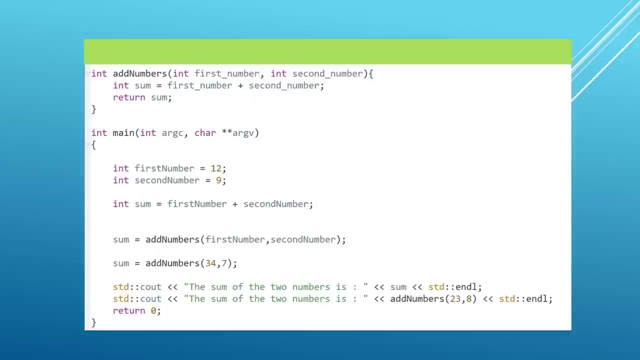 You're going to see how this works in a minute. A function must be defined before it's used, So you can't really call a function You haven't defined first In your C++ program. And here is a slightly complete program. 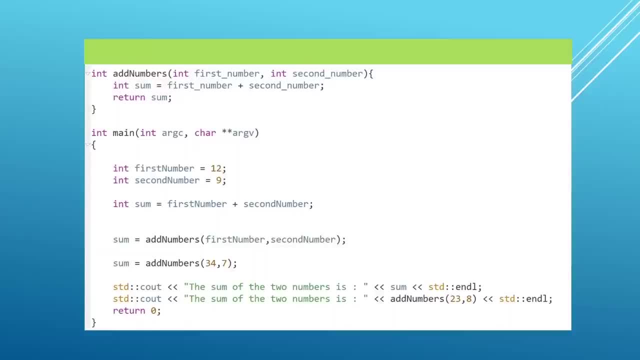 To really put all these ideas together, We have our function to add numbers. It takes two numbers And second number. It's going to add them up And store the result And we're going to return sum To be used by whoever called this function. 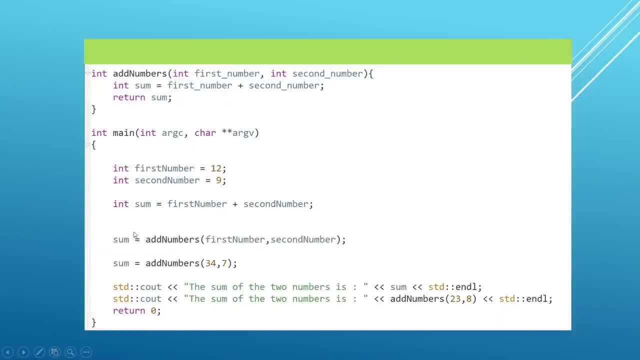 And if you look in our main program, We have a statement here. We're going to store the result Of add numbers In the sum variable And we pass first number And second number in the function And we're going to have that result stored in here. 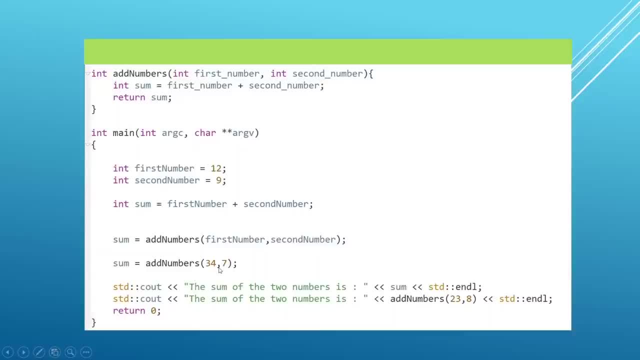 Here we also call the function With direct numbers In 34 and 7.. And we're going to print out the result here. This is the basic idea I want you to have about functions. They are reusable pieces of code That group together a bunch of statements. 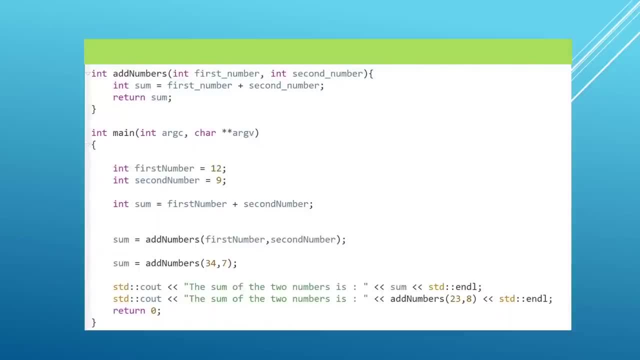 To do whatever it is We want to do in that function. One benefit about functions Is that we can reuse the code here. If you look here, We are calling this function multiple times Without really rewriting these statements That are inside the function. 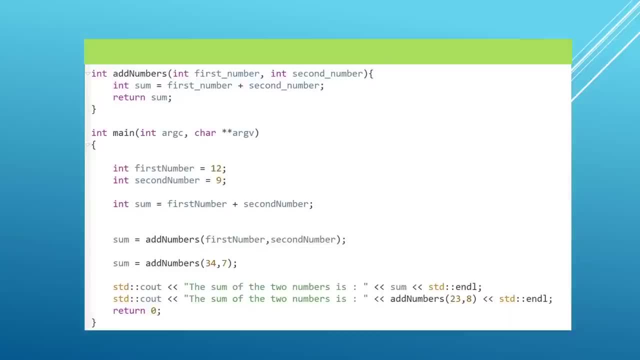 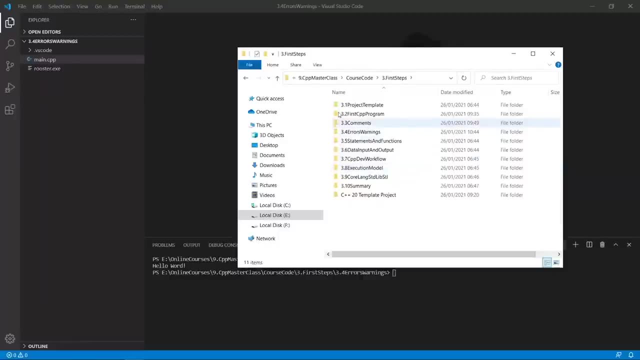 I know some of these concepts, But I want to show you How it works. We are going to go to visual studio code And try this in code And you're going to see exactly how this works. Here we are in our folder. 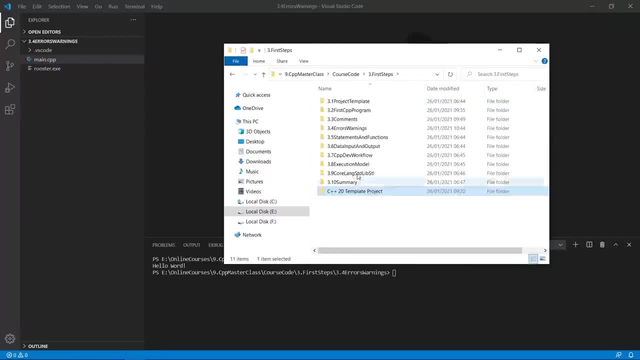 Where we are storing our projects. I am going to grab the code from the template project. I am going to put that in the current project, Which is statements and functions. I am going to paste that in here And I am going to open this up. 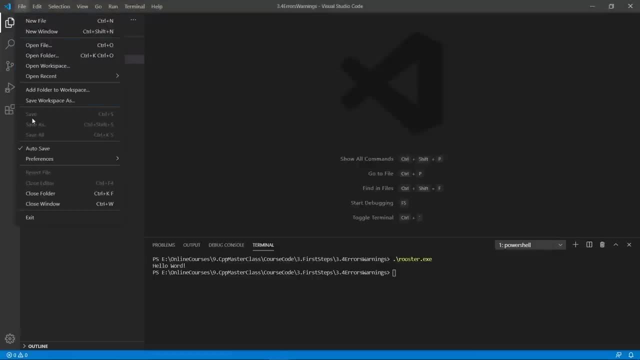 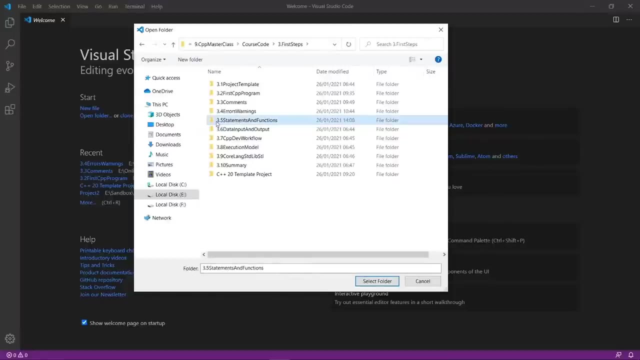 In visual studio code. I am going to close the project we have right now And I am going to open Our new project. Let's browse to its location. I am going to open the project On statements and functions. Let's open this folder. 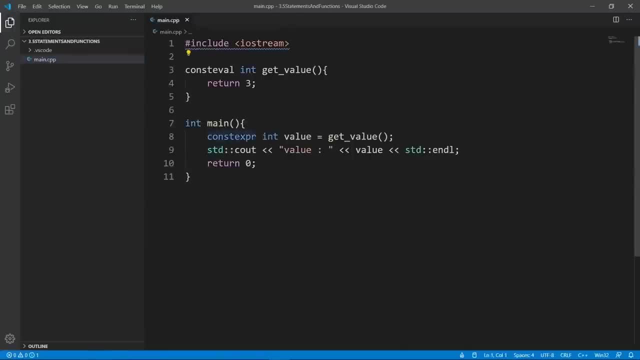 In visual studio code And we are going to have our starter project here. I am going to take out whatever we have in the main function And take out this const eval thing- We don't really need it- And we are going to try and define two variables. 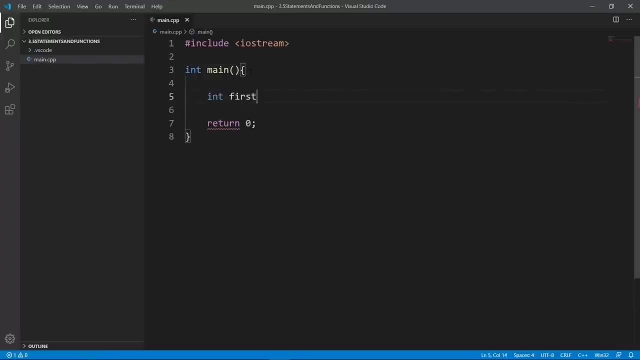 Using two statements. We are going to say int, first number, And we are going to put in a value, Let's say 3. And we are going to enter this with a semicolon. So this makes our statement. We can encode this in a comment. 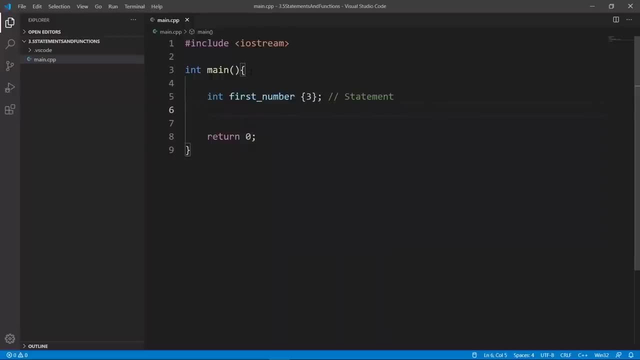 To make this pretty clear: We are going to also define a second variable. So we are going to say int to Mean that it is a whole number. It doesn't have decimal points Like 2.5.. It is a whole number. 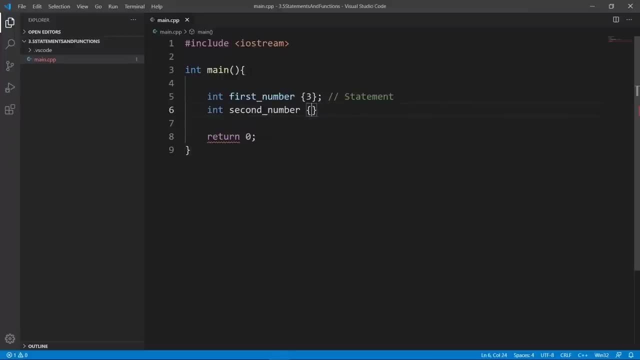 Like 1 or 7 or 10.. So we are going to say: second number, We can give it a name And let's put in a 7. And we can print these values out. Let's print them out first. So we are going to say: 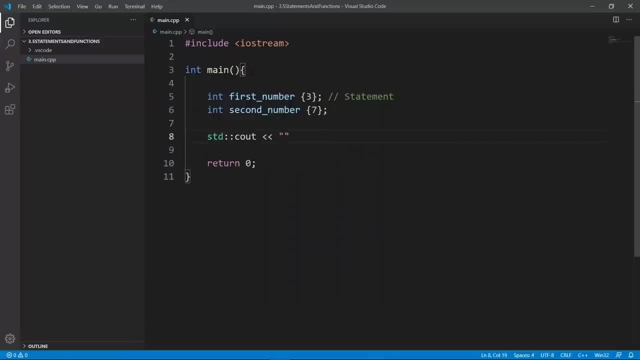 stdc out. We already know how to do that And we can say first number And we can change these output statements And say: the first number is first number. You can do that, stdendl, And you can notice that Visual Studio Code is really helping out. 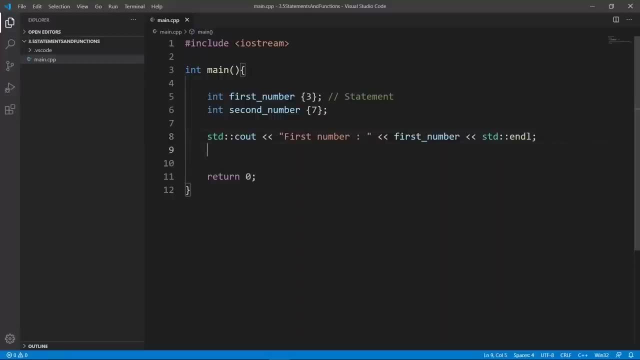 In auto completing Things we have in our program. Let's print the second number. So if we do std, You are going to see that It is going to give us a bunch of options We can choose from If you want. 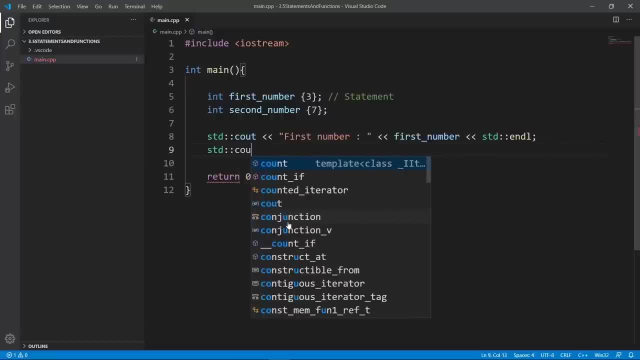 You can scroll through this with your mouse Or you can just type whatever you want to type. So I am going to do cout And it is going to try and help out. If I really want, I can come on cout here And click on it. 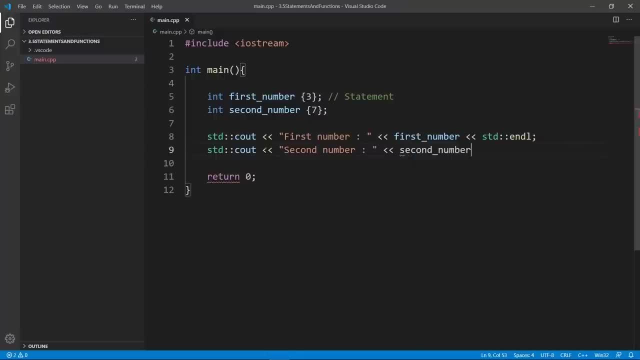 And it is going to be auto completed, Which is pretty cool. So we are going to say second number stdendl And we can try and compile this program. Before we do, I want you to guess what we are going to get When we run this program. 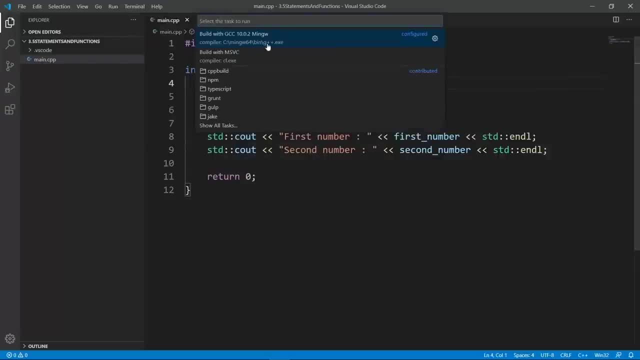 Give it a guess. We are then going to go to terminal Run task And we are going to build this with gcc. The build is going to be successful. We are going to open this in our terminal. The terminal goes away, No problem. 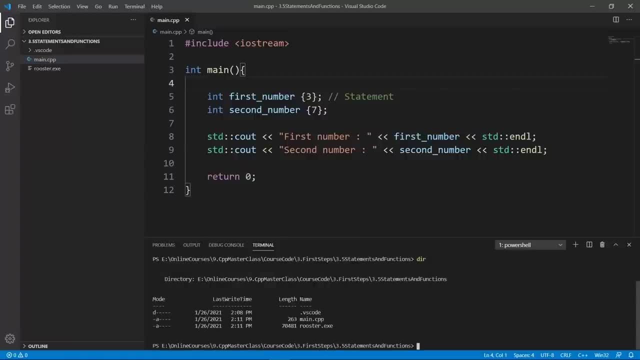 We are going to open it again And you are going to see that we have roosterexe, Our program. We can run it And it is going to say first number 3. And second number 7.. This is what we have stored in these variables. 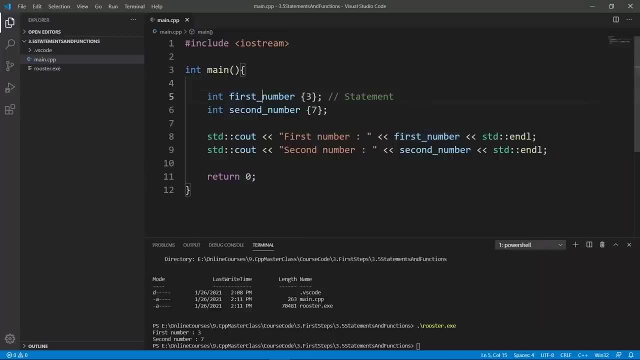 And the benefit of storing your data In variables Is that you can change the variables And let the rest of your program Really do the same things And pick up the data that you have in those variables. For example, We can put 13 in the first number. 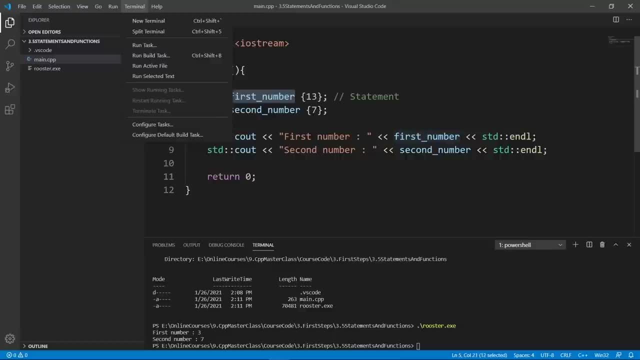 And if we build again, This number is going to be picked up by this code And we didn't need to go in And manually change data In these stdc out statements. here Let's build So that we can say this: 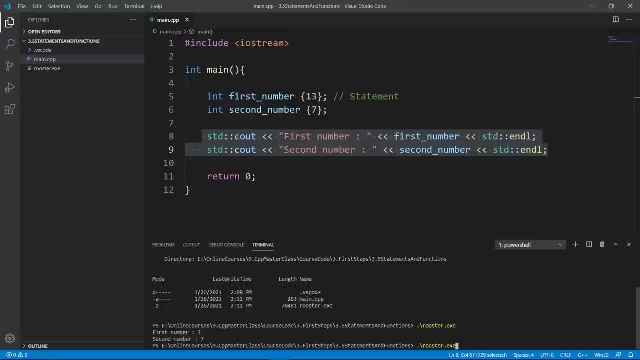 And we can close this by clicking, And if we run rooster again, It is going to say 13 and 7. Play with this a couple of times Until you really feel confident, And if you have any problem, Don't hesitate to ask me. 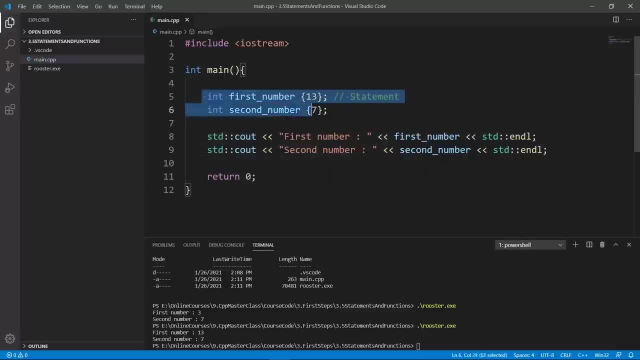 I am going to do the best I can to help you out. Now that we have these numbers Stored in our program, We can add them up. Let's say and sum. We are going to declare another variable And we are going to say it is equal to first number. 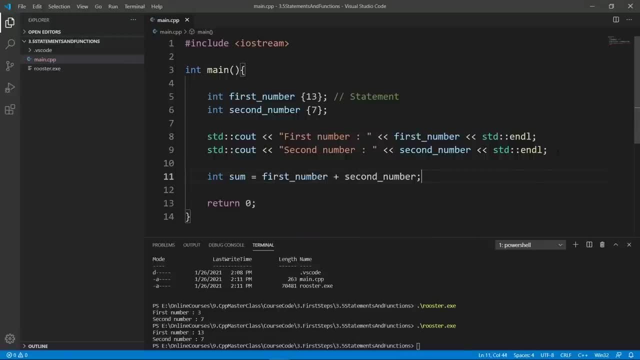 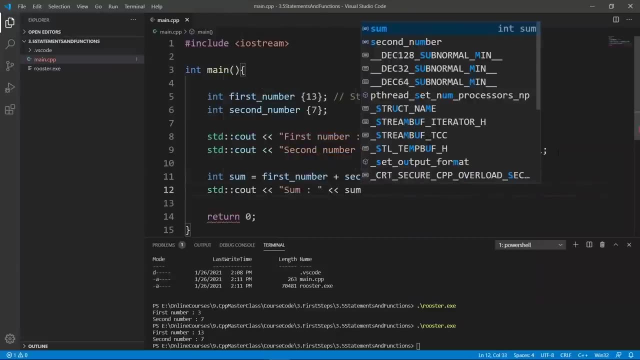 Plus second number, And we are going to end this with a semicolon And we are going to print the sum out- Let's do stdc out- And we are going to say The sum is sum. We are going to print our variable here. 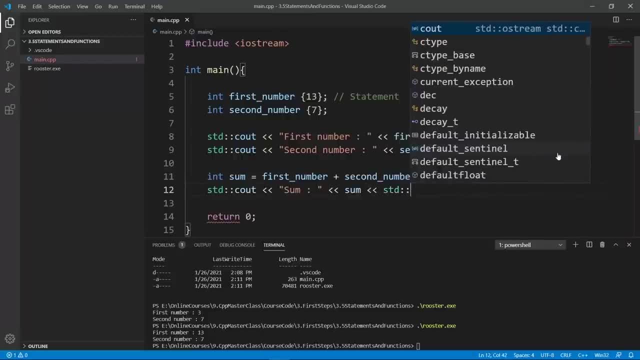 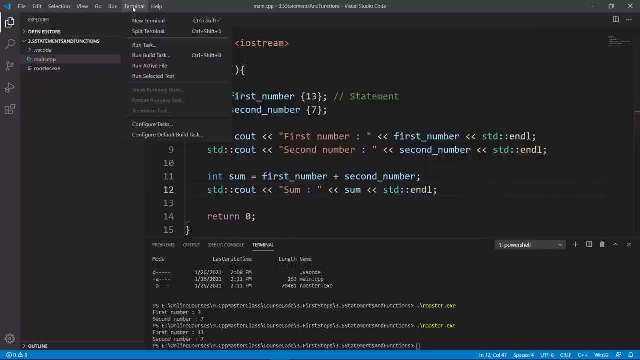 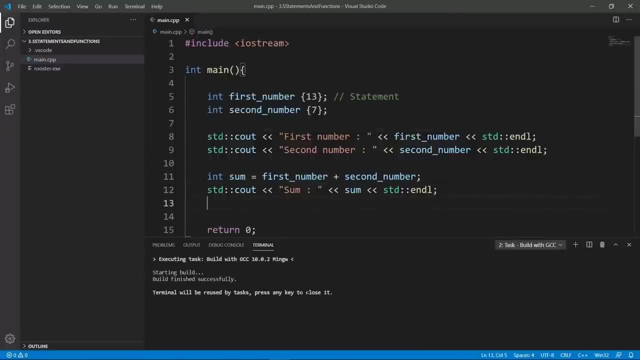 And we are going to print a newline character With stdendl. We are going to build our program So that our changes are reflected In our binary here. So we are going to go to terminal Run task Build with gcc. The build is going to be successful. 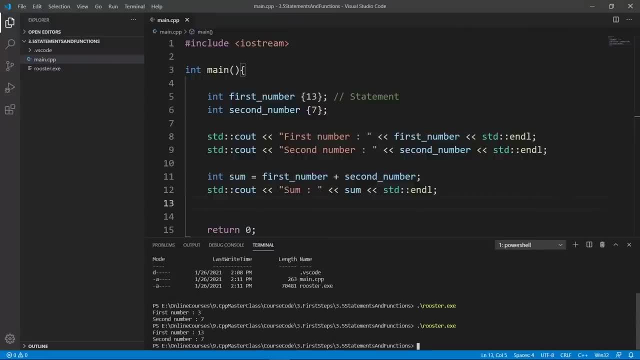 We are going to press any key, We are going to click here in the terminal And we are going to hit enter And run rooster again And we should see the sum. And you see, it says the sum is 20.. Which is what we expect. 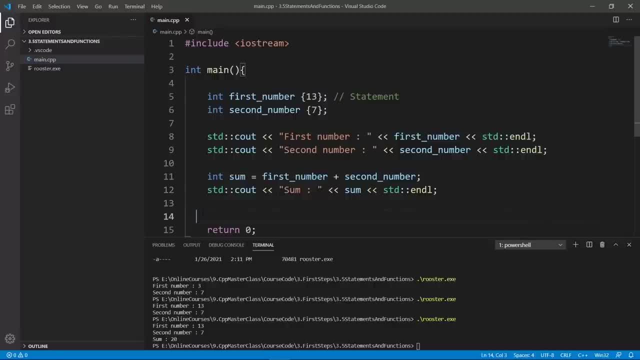 Now we are doing the sum here, And it would be better if we are not doing the sum In the main function here. What if we actually took this code And wrapped it in a function That we could reuse whenever we want? We have seen how we can declare a function. 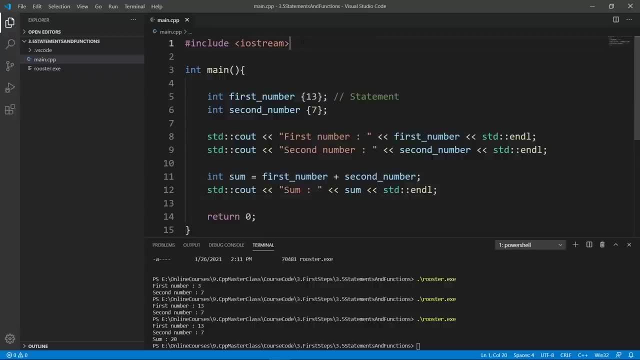 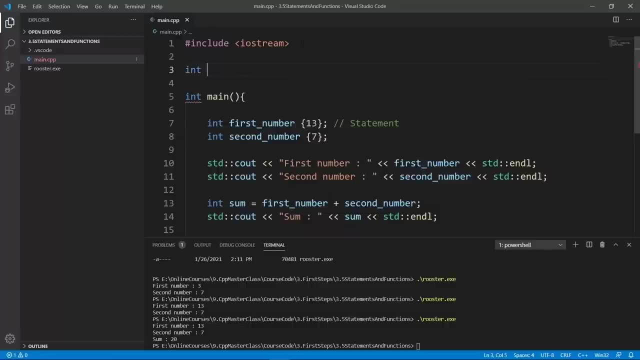 So let's do that. We are going to follow the same structure We saw in the slides earlier. So we are going to say int- This is going to be the return value, Or what we get out of the function. Then we are going to put in the name of the function: 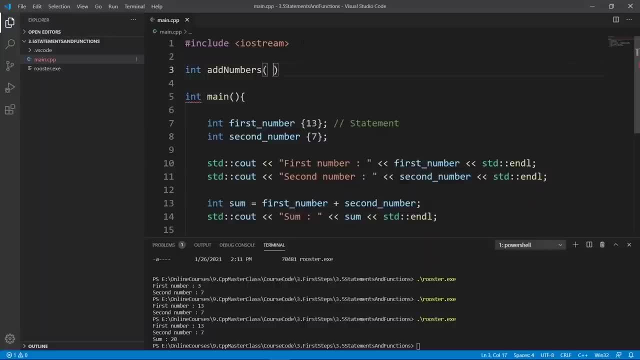 We are going to say add numbers And we are going to pass in the parameters. The parameters can really have any name you want, But you have to specify The type of the parameter first. So the parameters are also going to be whole numbers. 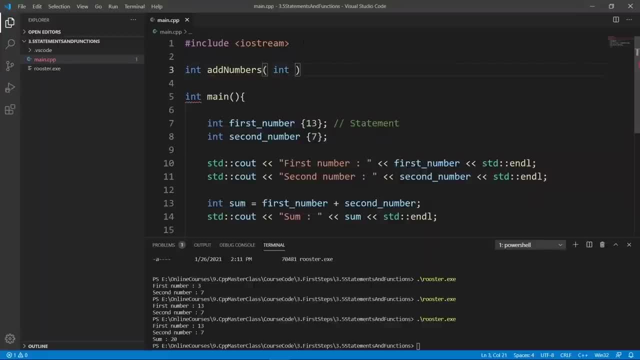 Like 1,, 5,, 7. Or whatever you want, And we are going to say first param And the second is going to also be a whole number, An integer, And it is going to be second param. Okay, After we do this, 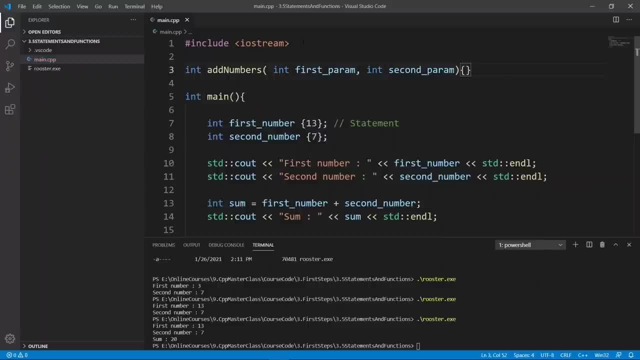 We are going to specify the body of the function Which is going to be between these curly braces. I am not going to do that. I am going to jump to the next line So that this is really easy to see. So I am going to define our sum variable. 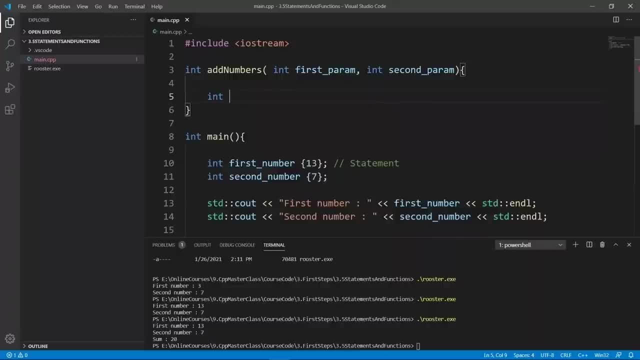 Inside the function It is going to be a whole number And I can call it whatever I want. So let's call it result, Because it is going to be the result Of this function And the result is going to be the sum of first param. 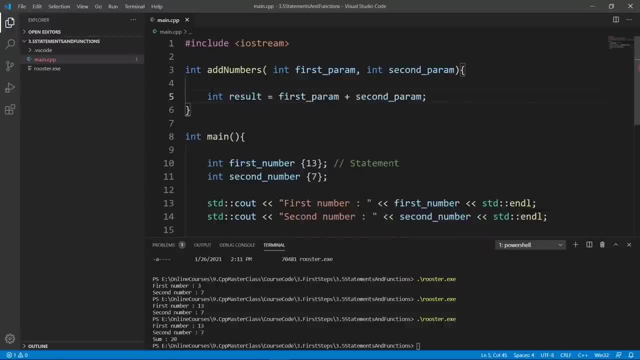 And second param. Okay, I hope this makes sense, And we are going to end this with a semicolon, Because every statement in C++ Has a semicolon. After we have the result, We need to give it back to whoever called this function. 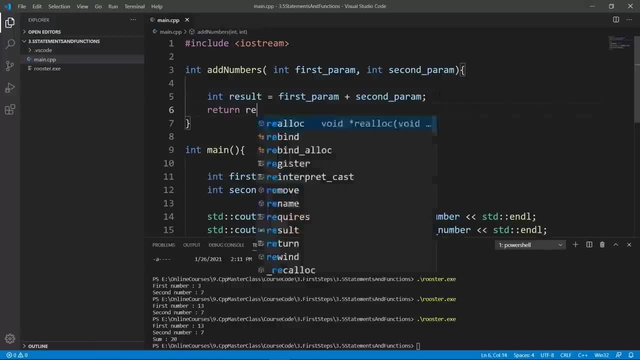 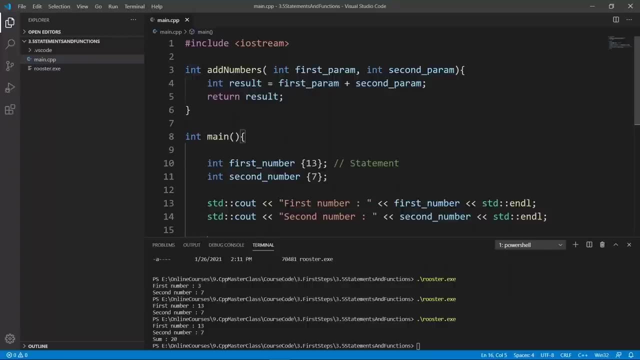 And we are going to do that With a return statement And we are going to return the result To whoever might have called this function here. Now that we have the function, We can actually use it. We are going to go back in our main function. 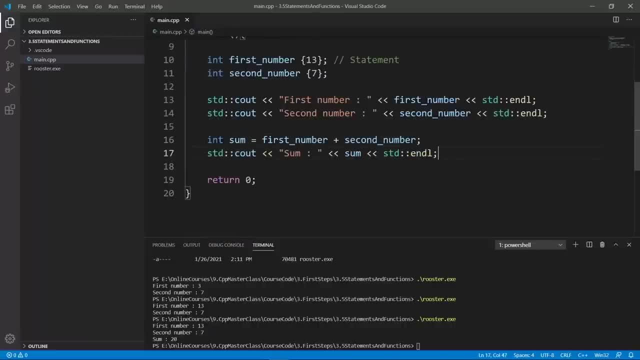 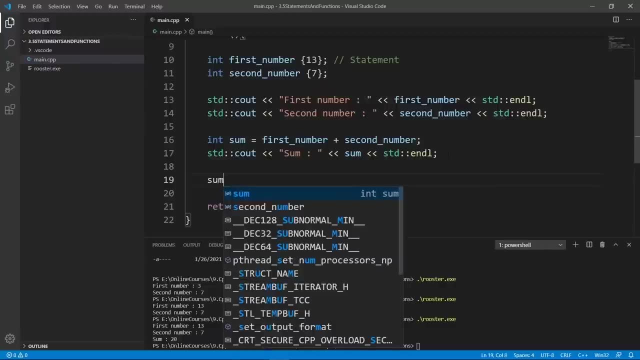 And what we are going to do Is to reuse this sum variable And store in Whatever is returned from our function, The syntax for that. This is going to be sum, And we are going to say equals And we are going to say add numbers. 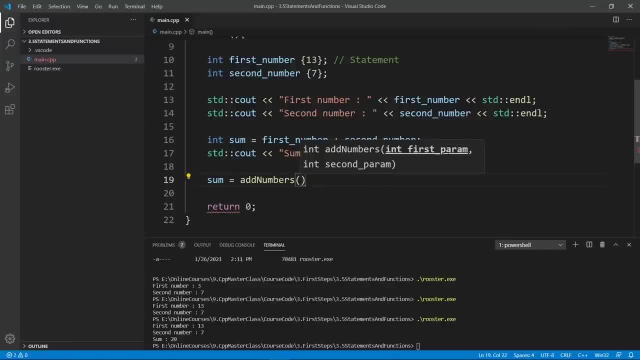 And we can pass in whatever two numbers That we want to add up. Let's pass in 25.. And 7, for example? We would expect this To give us 32.. So if we print the sum again, We can just copy this statement. 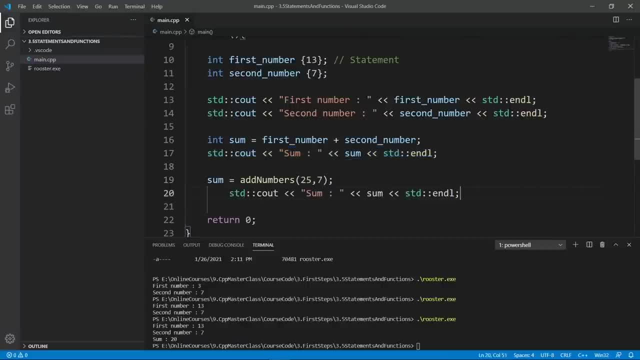 That prints the sum And reuse it here. Let's align this a little bit And I want you to take a guess At what we are going to get From this program. right now We have these two numbers. We are adding them up. 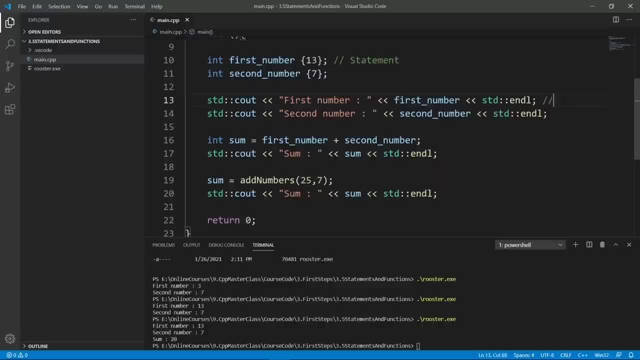 If we get here, This should print the first number, Which is going to be a 13.. So here we expect to get 13.. And by the time we hit this second number statement, We are going to print the second number. It's going to be 7.. 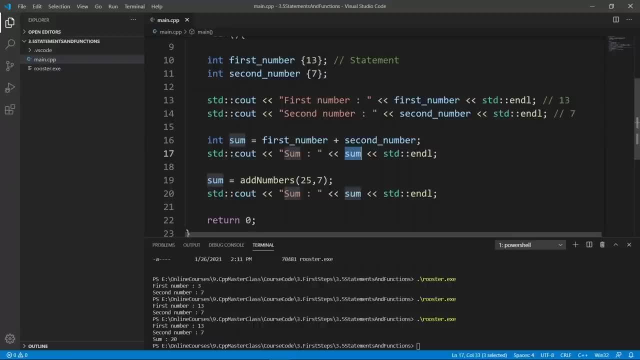 If we get here, We are going to print whatever is stored in sum, And in sum We are going to print the second number, So this should print 20.. And here we are doing another sum Of two numbers, But we are using a predefined function. 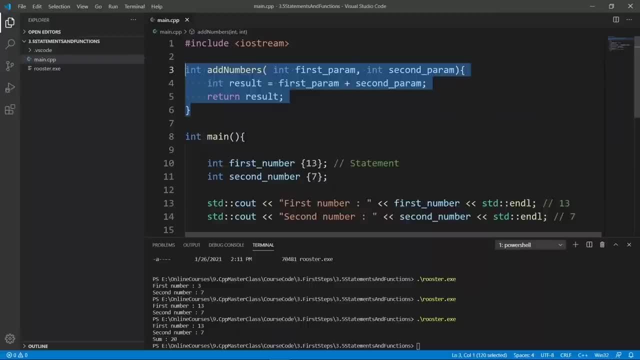 That we have here Before the main function, Because you have to define the function Before you use it. If we add 25 and 7. We are going to fall into this function And it's going to add those numbers up. 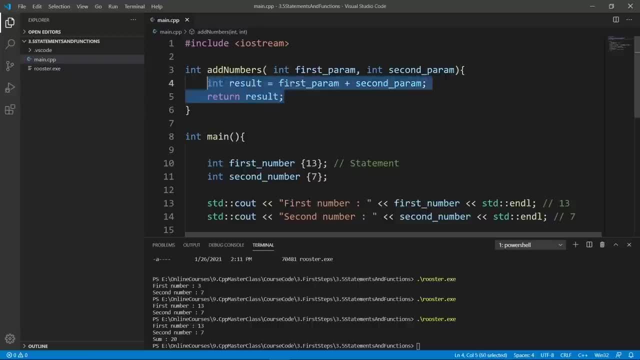 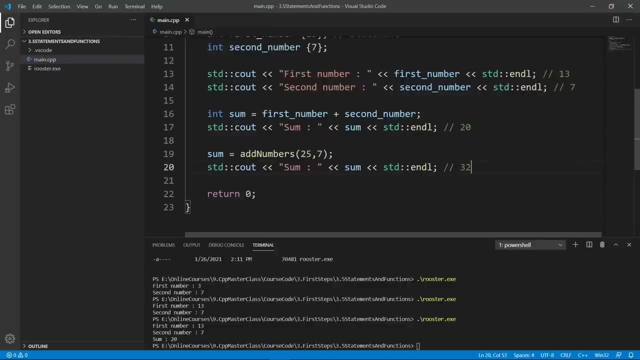 And we are going to get 32 in here And that's what we are going to return And it is going to be saved This variable. If we print it out, It's going to give us 32.. I hope this makes sense. 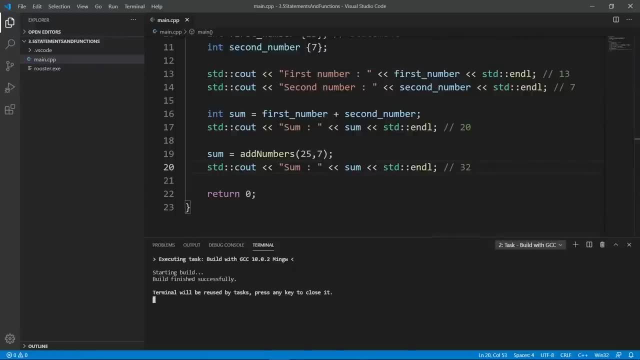 Let's build and run our program, Run task Build with GCC. The build is going to go fine. We are going to go back to our terminal here. Let's clear So that things don't disturb us And bring in some confusion. 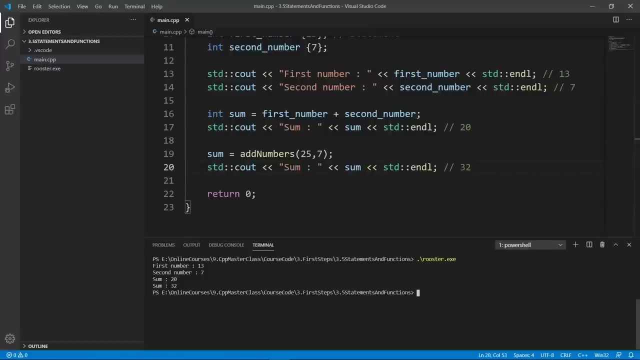 We are going to run our rooster program And exactly what we have here. We have a 13 from the first statement here, We have a 20 from this sum here, Which is here, And we have a 32.. That we got from this function. 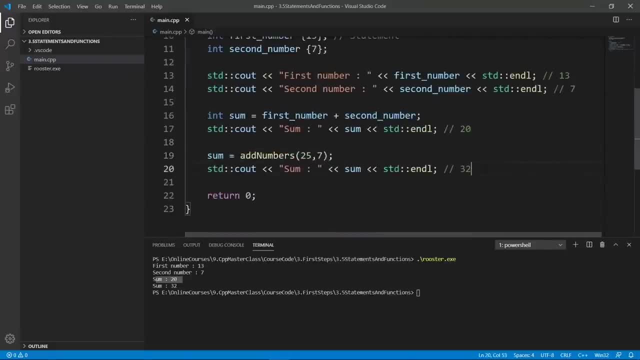 The good thing about functions Is that we can reuse them. Now that we know how to use it, We can use it again And we can say sum equals, add numbers. And we can say 30 and 54, for example. You add them up. 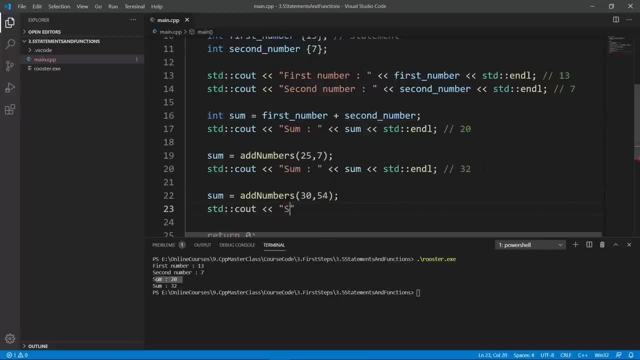 And you are going to get the result. So we are going to print the result Sum. I really want you to take some time And play with this statement So that these things make sense. It's really not that difficult, But you just have to wrap your brains around. 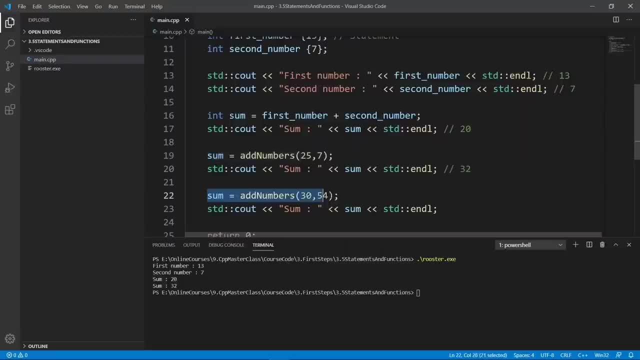 How C++ defines these things. So we have this statement And we are adding 30 and 54. So it should get an 84.. After the 32 here, Let's build. We are going to run the task To build with GCC. 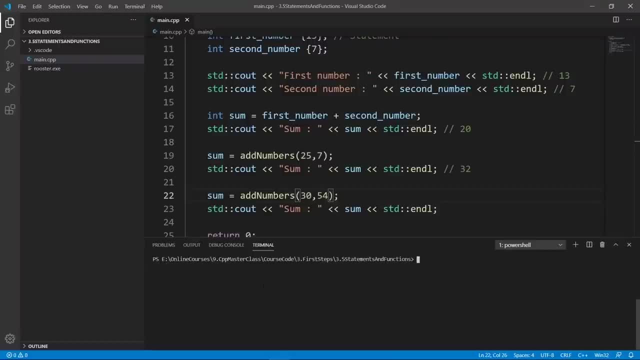 We are going to click on the terminal here And hit enter. We don't have things disturbing us And we are going to run our program And we have our trusty 84 here. I really hope this makes sense And as a bonus, 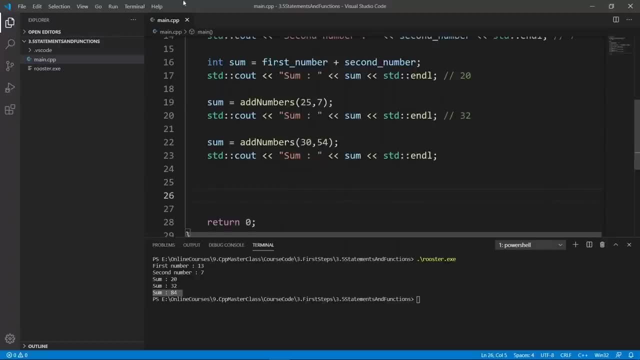 I am going to show you That you can also call things In the std cout statement here Without having to store them In some predefined variables, And sometimes this comes in handy. So you can say std cout And we are going to say sum. 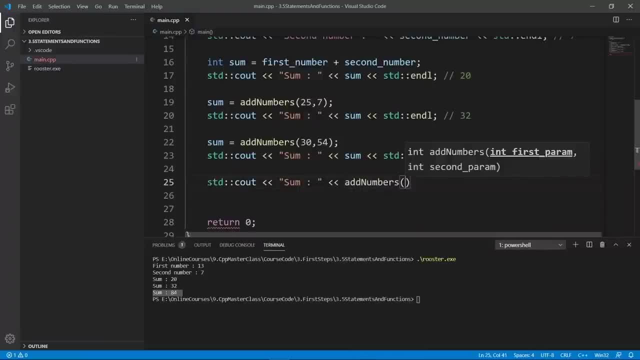 And you might say: add numbers Right in here And you are going to say 3, for example, And 42. And this is going to give us a 45. That's what we should expect to see After 84 here. 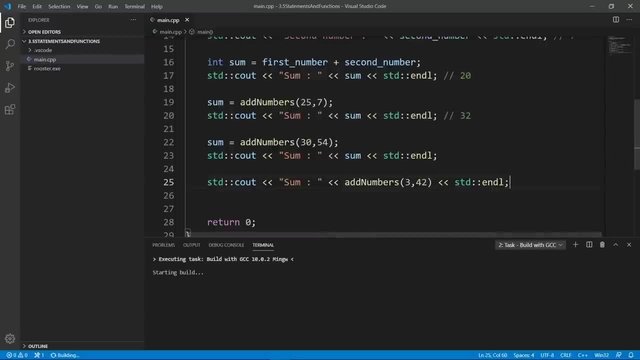 So let's build And run the task to build with GCC. The build is going to be successful. We click on the terminal here. We hit enter So that we see our terminal with output. We are going to clear So that we see our output without noise. 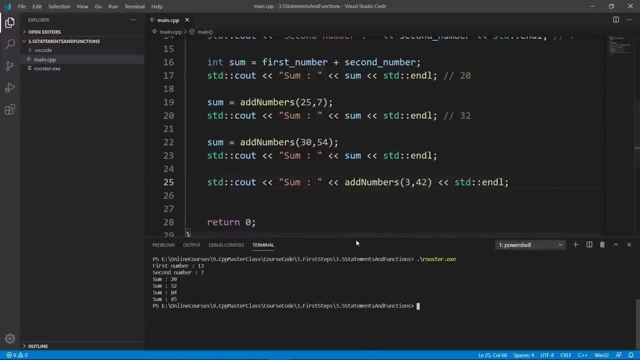 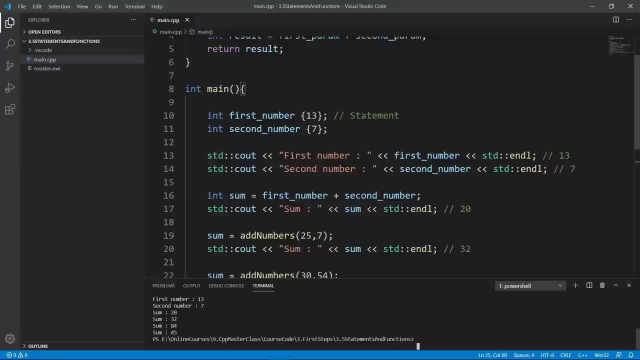 We are going to run our program And run the task. I hope this makes sense. The whole point of this lecture Was to make you aware of statements And function. A statement is the most basic unit In your C++ program. 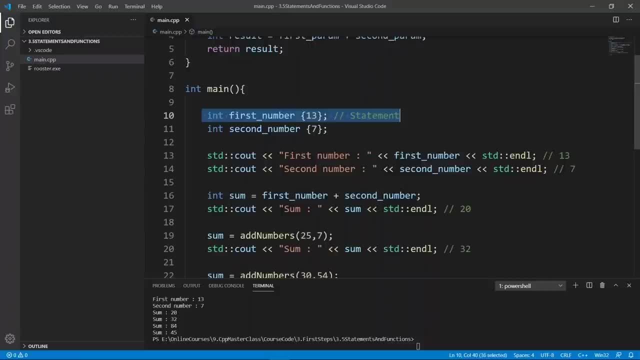 It basically lives on one line, But it can also spread across Different lines, But we are not going to look at that here. Maybe we are going to see that later in the course. Statements are executed in order, So when our main function gets to be run. 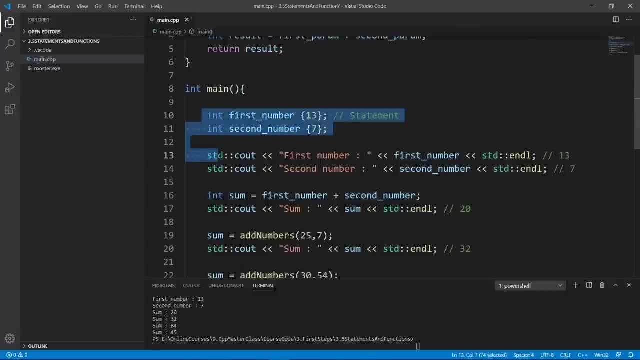 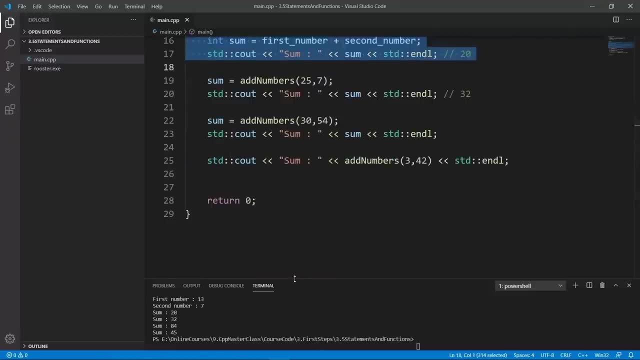 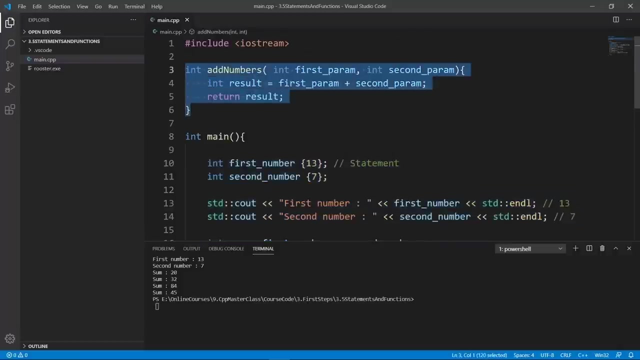 By the computer. second statement, third statement, and it's going to go until it hits the end and we can see that here, in the order in which our numbers are printed, it is going from top to bottom. We have also seen that we can split our code in different functions and wrap whatever functionality we have in a 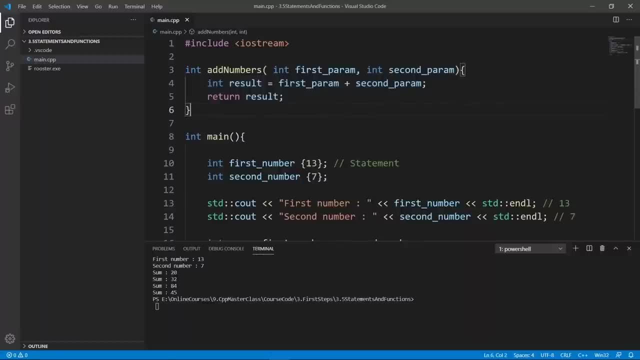 function. We have seen the basic concepts on functions. A function has a return value, it has a name and you have to give it the parameters and you put the body of your function within these two curly braces. As an exercise, I would challenge you to do a function that multiplies two numbers. 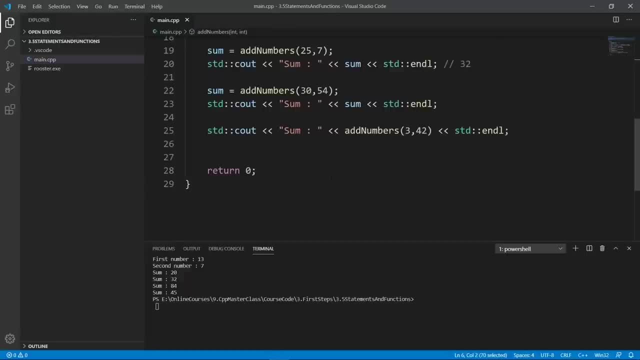 and call it in the main function here to see the result. If you have any problem, please do ask me. I am going to do the best I can to help you out. This covers all we set out to do in this lecture and I hope you found it interesting. We're going to stop here in this lecture and the next one. 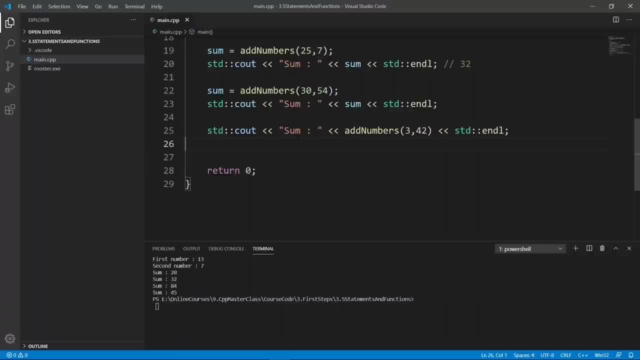 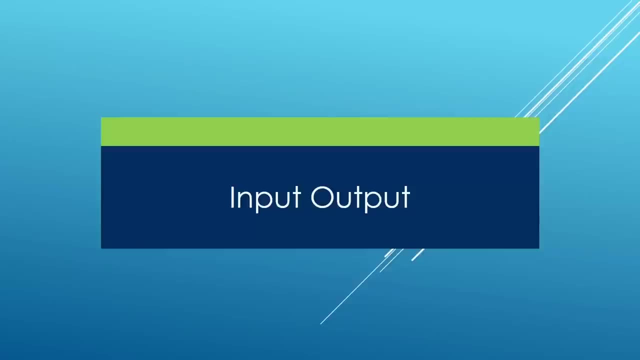 we're going to see how we can input and output things from our C++ program. Go ahead and finish up here and meet me there. In this lecture we're going to learn about how we can get things in our program and get things out of our program, and that's basically input. 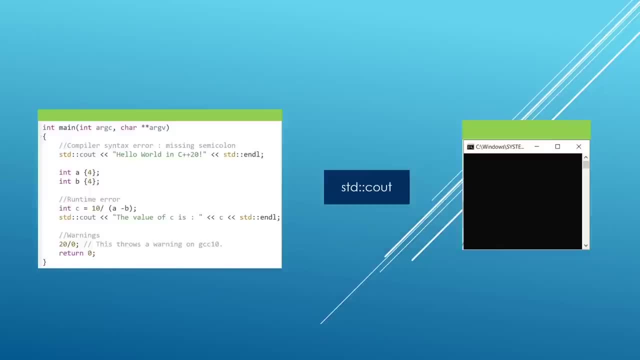 and output to and from our program. We have actually been doing this all along. We have been printing things from our program to the console and with this technique you can really think of stdc out as a highway that goes from your program to the terminal. 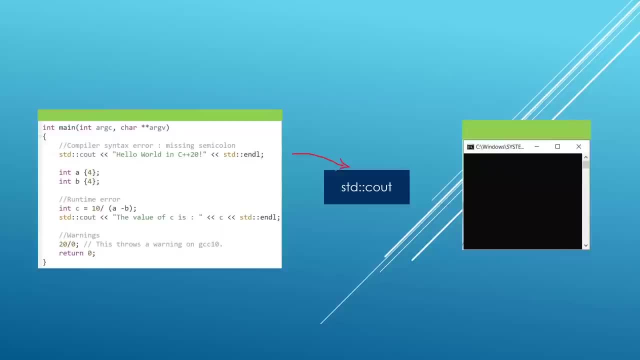 You can basically think of it like this: Data is going from your program to stdc out and it's going from here to the terminal and from this you might get an idea why these less than signs kind of point to the left. because data is going from your program to stdc out and these two symbols 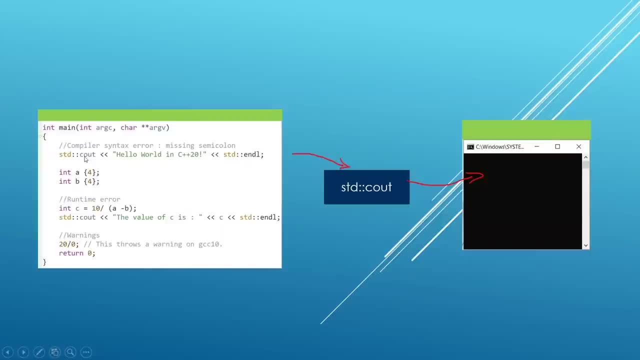 point to the left. They point to stdc out, to signal to the fact that data is going from here to here. I really hope this makes sense, because sometimes these things can confuse people. This is the reason why it's going from your data to stdc out. Data is basically going. 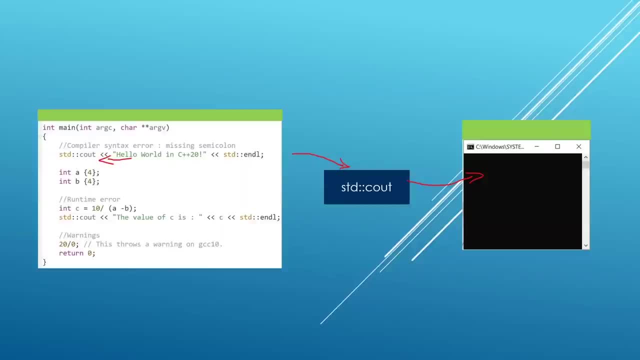 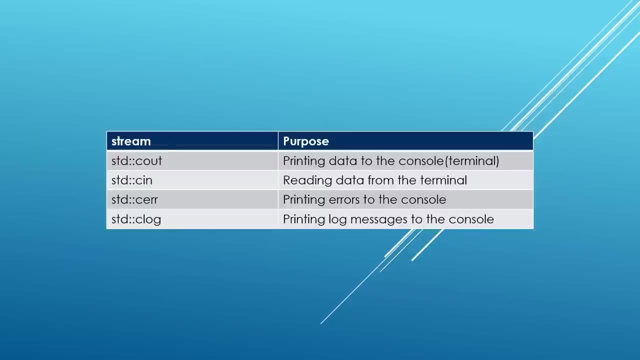 from your program into stdc out, and stdc out is one way we have to get data from our program to the console. There are many others. We have stdcerr, or stdcerr- This is what I like to call it- and what it does: it prints errors. 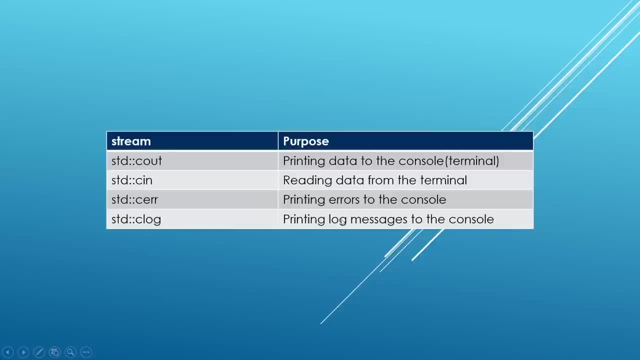 to the console. We have stdc log, which is going to print log messages. Why do we have these different things? Different programs might decide to format these messages differently because they are different messages. One is a simple message from the program, Another is an. 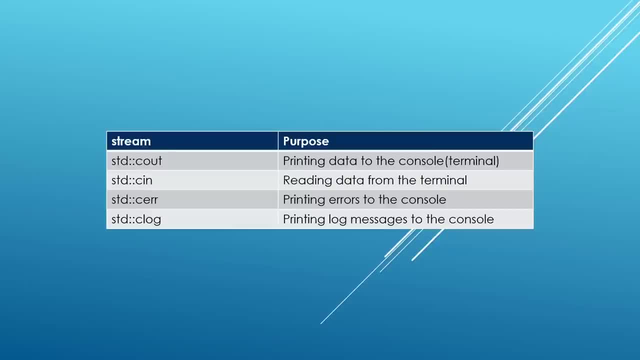 error. You might want to turn this red to really bring the attention to this message, because the user has to solve that problem. Another might be a log message that you want to store in some file or some database. You might want to store it in a folder, or some folder and store it in a folder. 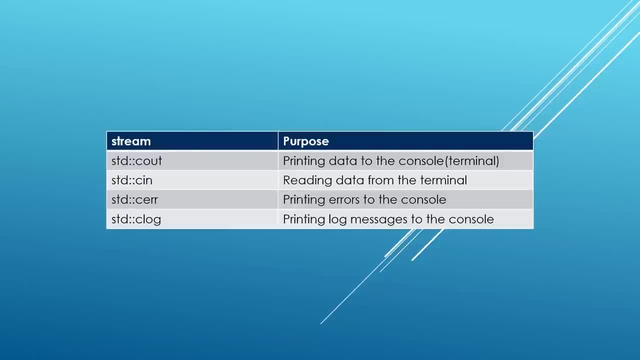 or some folder and store it in a folder. and store it in a folder. and store it in a folder or some database. Users for these things differ and C++ makes sure to give you different ways to state your intent through the tools that you use. We have looked at stdc out, stdcerr and stdc log. 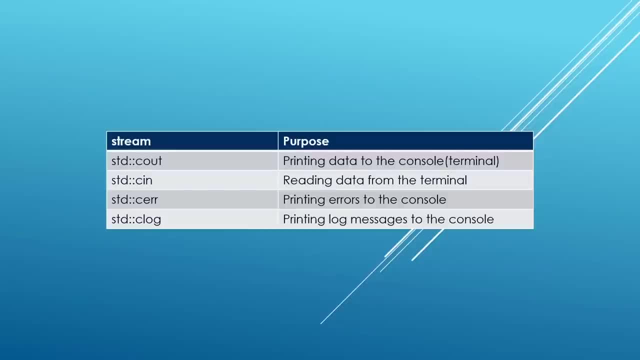 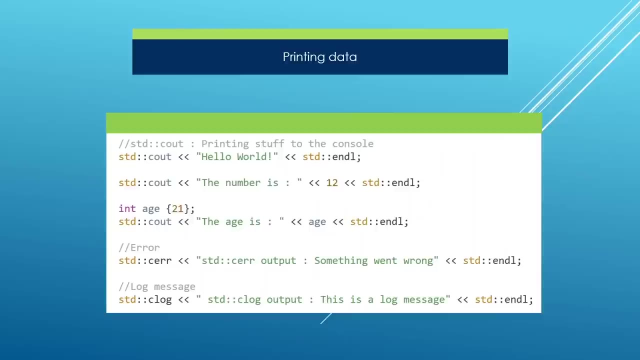 What does stdcin do? It does the reverse: It's going to take data out of the program and bring that into the program. So let's look at a few examples using these. Here we have an example of printing data from the program to the terminal through cout, cerr and clog. Here we have a hello. 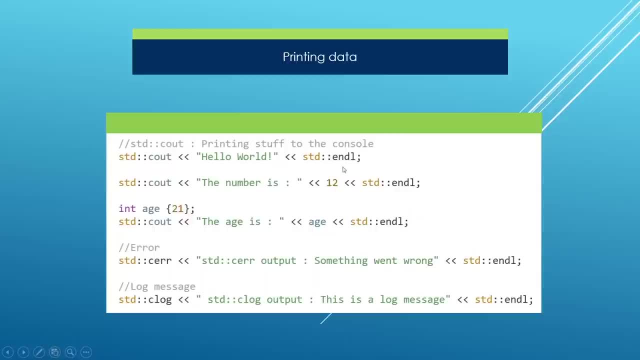 world message going to cout. Here we have a number going to cout. This is what we've been doing all along. We can also do a variable, storing the edge, For example. it's a whole number, It's an integer. So we print this out and the message is going to go from the program to cout. So you can think that. 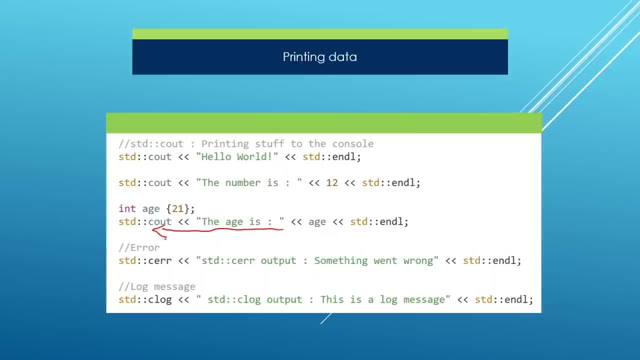 things are going from the program to stdc out. I really wanted this to make sense. Okay, if we go down, we're going to see that we can use cerr to print errors to the terminal and we might say something went wrong or something along these lines, to bring the attention to the problem And 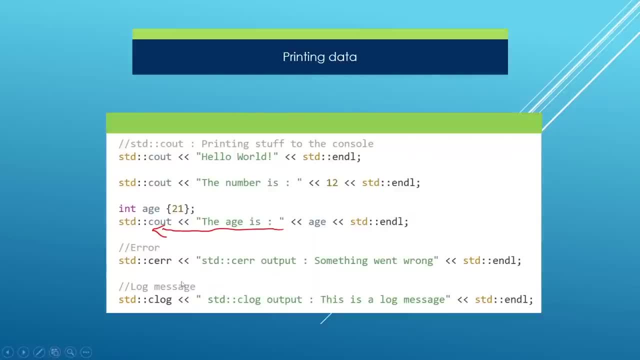 we can use clog to print log messages and they work the same way. They all use the stream output operator and it is going to take data from the program to the output stream. really, This is what we mean here. Here is an example of how you might read. 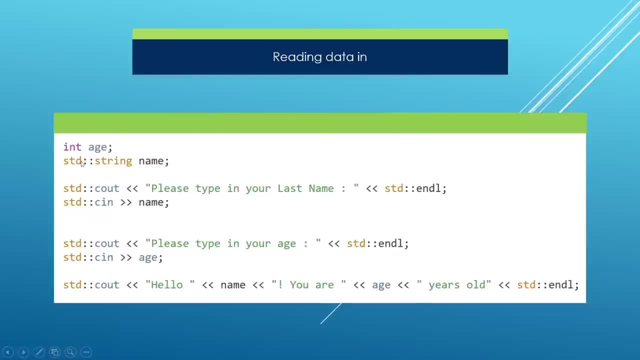 data and bring that into the program. Here we have two variables. One is the age- It's a whole number or an integer in C++, and the other is a string. This is a type that allows you to store strings in C++. We're going to learn a little more about this later, but here I want to use it to really 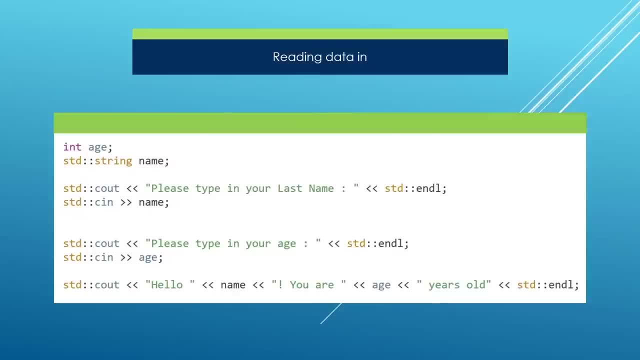 make it clear that you can get things from the outside and bring that data in your program. So we're going to let the user type in the last name And this statement here with CIN is getting data from the stream or from the highway through which data comes into our 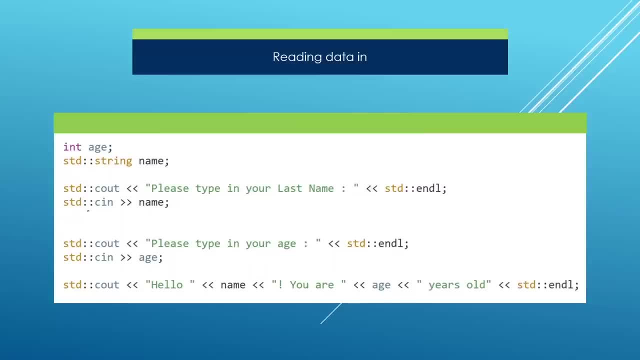 program and bringing that in our program. And here it should be clear that the flow of data is in this direction. Data is going from CIN and we're storing that in a variable that we have in our program that is called name. We do the same thing and ask: 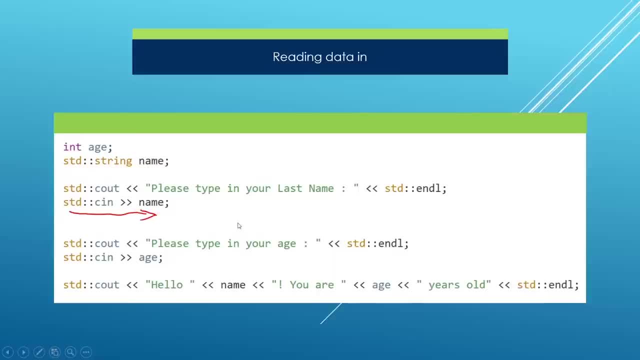 user to print the age and they are going to print that and the data is going to come from cin and we're going to store that in our age variable here after we collect the data from the user. we're going to print that and we're going to say hello. we're going to print the name and we're going to say: 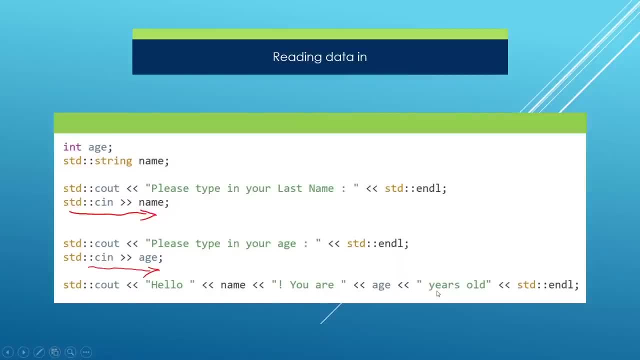 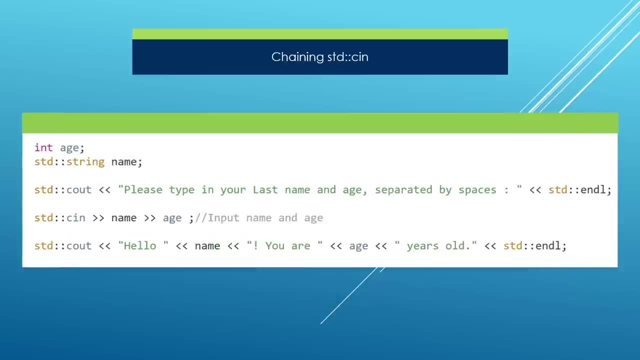 they are, whatever years old. this is what this program does and i really hope it makes it clear how data input works through streams in c++. another thing we can do with stdcin is chaining input, and we can use this technique to grab data in one statement. look at the program down here to: 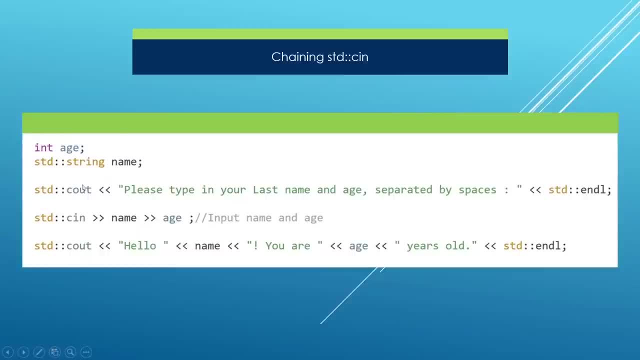 really understand this. we have the same variables- age and name. we let the user type in the last name and age, separated by spaces, and we grab the data like this: we first grab the name, after that we grab the age and we grab the data like this, and we grab the data like this and we grab the data. 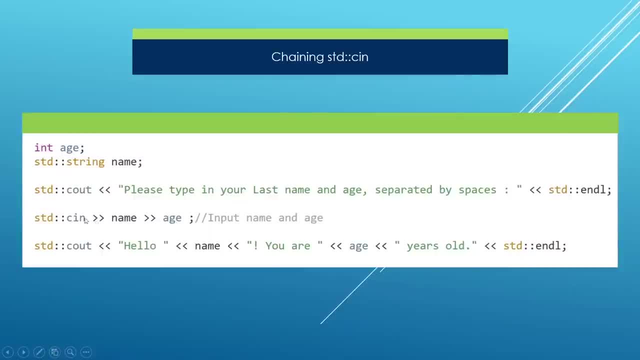 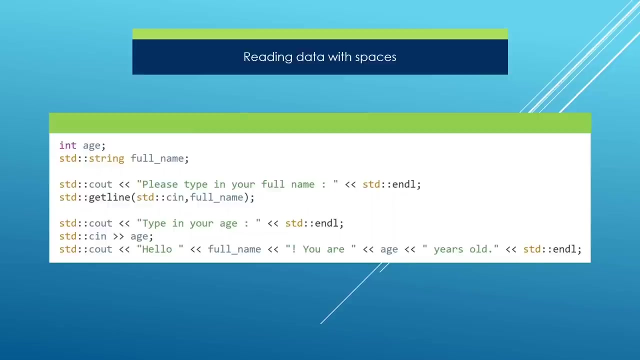 going to print the same things and we can chain input stream operators like this to grab the data in one go, and this may come in handy sometimes. before we try these things in a visual studio code, i want to bring your attention to a problem that you are likely to come in contact with, and 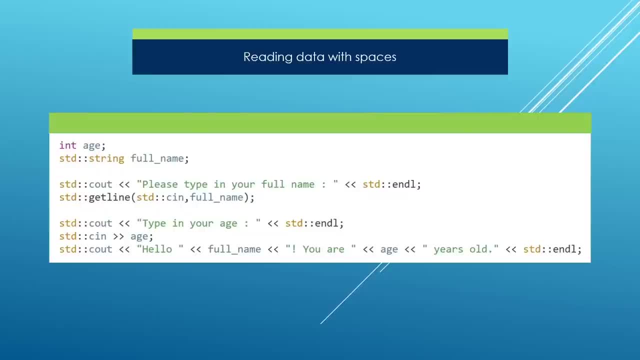 that is, reading data with spaces. what if the user types the name with spaces? for example, you ask me to type my name, i'm not going to type it. i'm going to type daniel capoia and your program is going to run into problems c++ allows to solve. 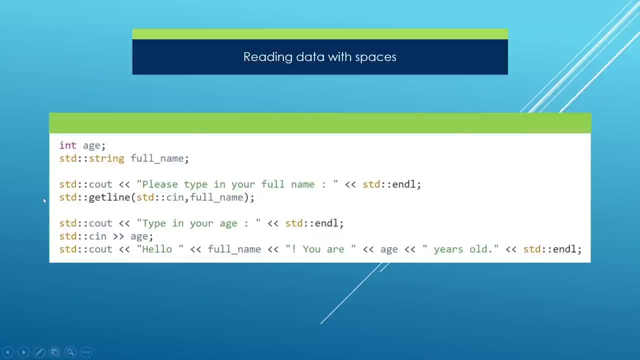 this problem using std get line and you use it. using this syntax, you're going to pass in the stream where the data is going to go and you're going to pass in the variable that is going to read the data and you're going to have this information stored correctly in your program. 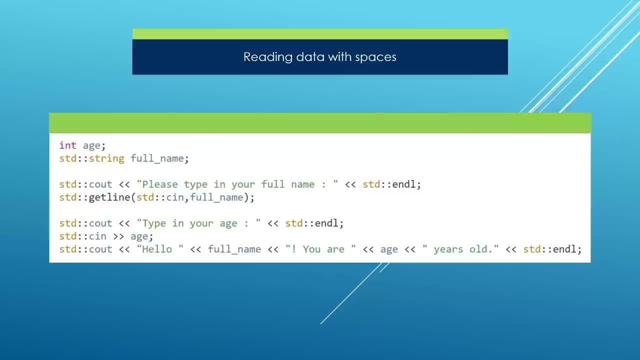 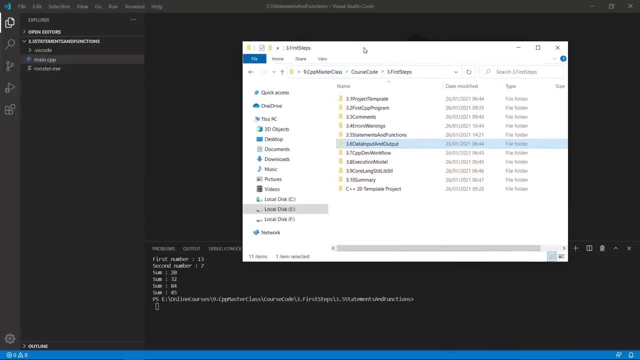 this might be not making sense yet to you. we're going to go to visual studio code and play with us, and i am sure it is going to make sense. okay, here we are in visual studio code and we have our project where we're going to store our files, data input and output. we're going to copy. 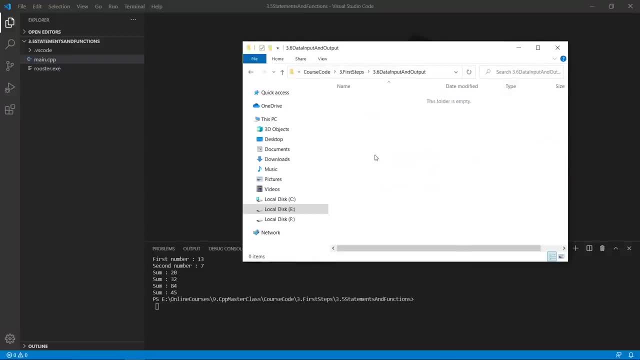 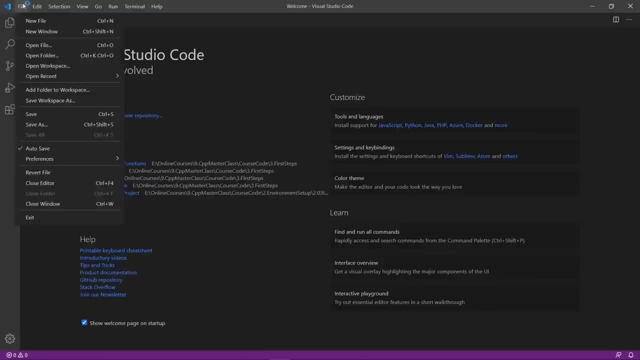 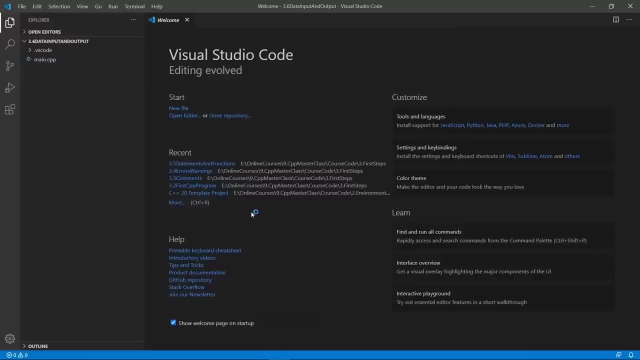 code from our template project and we're going to put the data in and i am going to open this folder in visual studio code. so let's close whatever we have now and i am going to open my folder. let's browse there. i am on this folder: data input and output. i am going to select that and 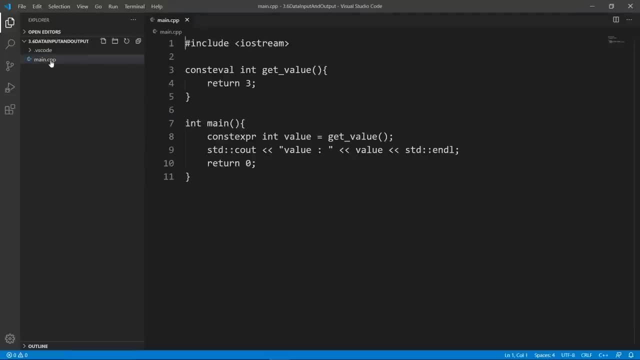 the project is going to open up in visual studio code. i am going to jump to my main function. i am going to take out things we don't need and the first thing we're going to do is printing data. we have really done this, so we're going to practice this a little bit. we can say stdc out and we can. 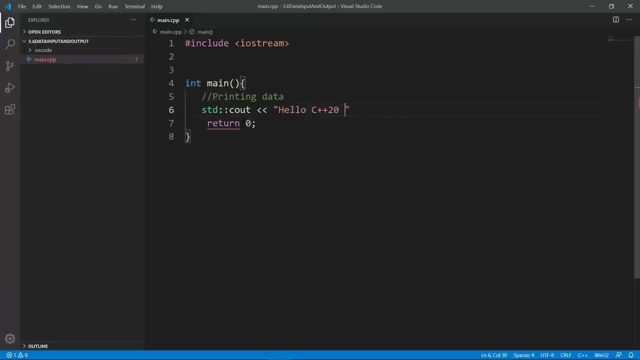 say hello, c++ 20, why not? and we're going to put an std endl at the end and remember our semicolon here and print our stdc. put in your head that data is going from our program here to sdc out and sdc out is going to dump that on the terminal. that's how this works. you can also do a variable. 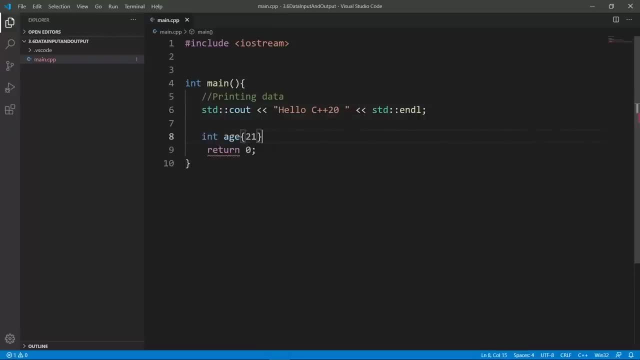 let's say int age, for example, let's say 21 and end this with a semicolon, and we can also print the edge, we can say sdc out and we can say age. this is going to be set to the output stream and we're going to do std and dl to add a new line character at the end and we can try and. 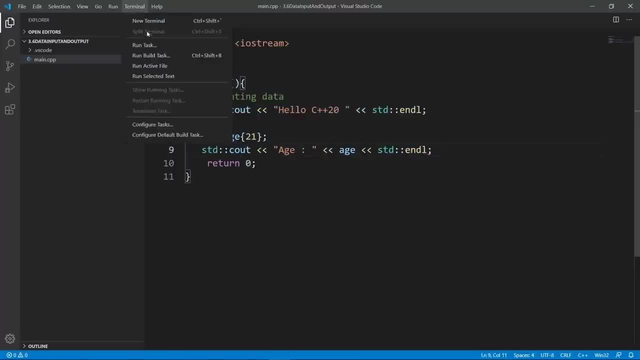 build this before the program gets more complicated. let's go to terminal. we're going to run the task to build with gcc and if we hit enter on the terminal here, the terminal is going to go away. we're going to create a new one, no big deal, and if we do there, we're going to find our rooster. 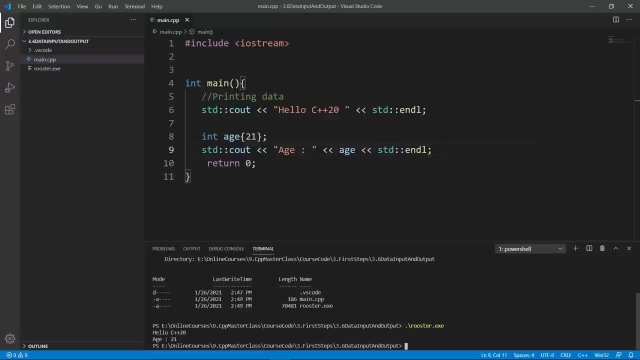 program. if we run it it's going to say hello, c++ 20 and the age is going to be 21. we are successfully taking data from our program and printing that to the terminal. this is pretty cool and you can think of stdc out as a highway that is really going to take your data from your program. 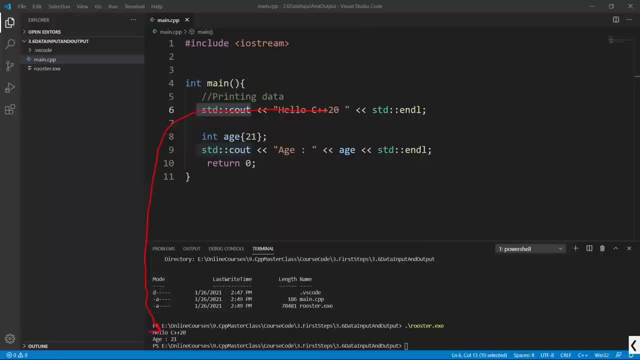 and bring that to stdc out. like this: we're also going to take the age it's going to go through stdc out and bring that to our program and bring that to our program. and bring that to our program. it's going to show up here. you can think of this like this: okay, now that we have used stdc out, we 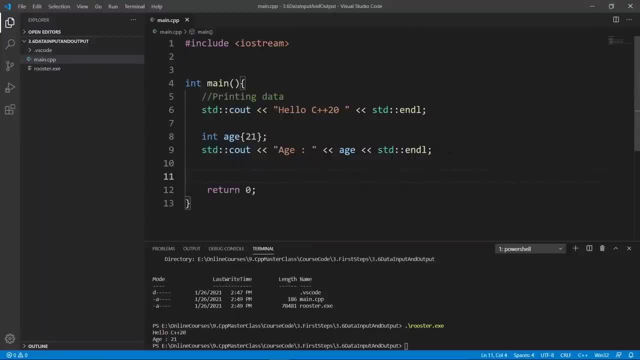 can use stdcr and std c log in the same way. so we're going to say std c r and we're going to say error message and the message is going to be: something is wrong. you may do whatever you want in here, and we have to remember to put a new line character, otherwise data is going to be cramped on. 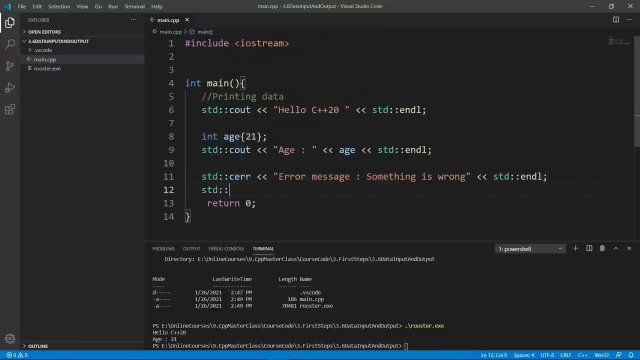 one line. we can also use stdc log. it really works the same way. c log and we can say log message and we're going to say something happened and we remember to put std endl and our semicolon. if we built this program, you might guess what it's going to do. it's going to print these things. 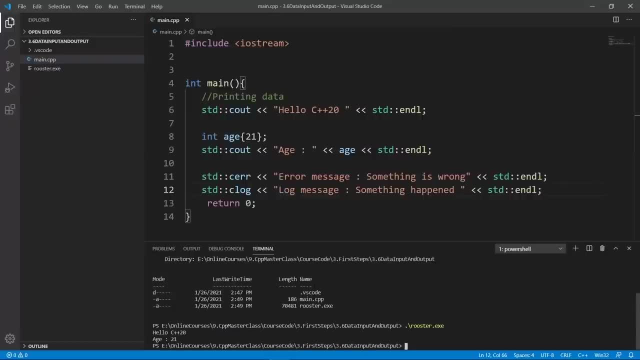 on the terminal, but this might be useful to terminal programs that support features to format different programs, to program the file that you use, which is what we're going to do with this messages directly. the program is going to know that one message is a simple message, the other is an arrow, the other is a log message. let's run our program. 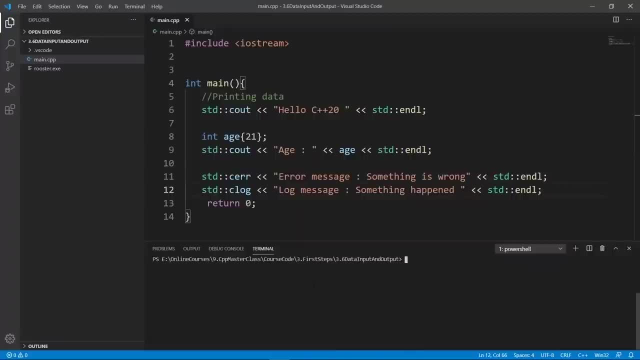 but before we do that, let's clear so that we don't have noise here. we're going to run the program and it's going to say the error message and the log message here. okay, now what we're going to look at is how we can get data into. 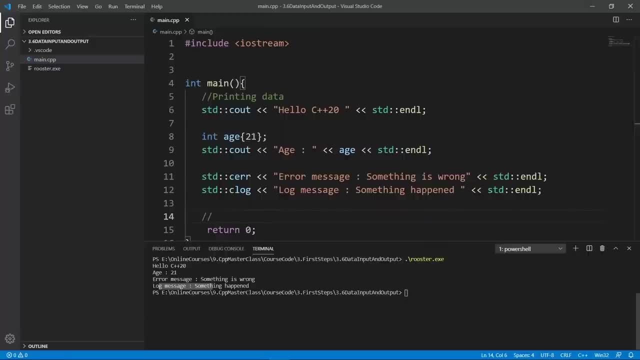 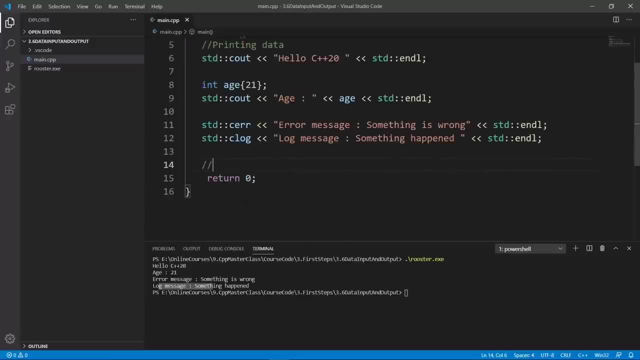 our program and data is going to be going in a different direction. it's going to be coming from the terminal and flowing into our program. what we're going to do? we're going to do and age one. this is a new variable, so we're going to put in data and we're going to bring in a string library to allow our 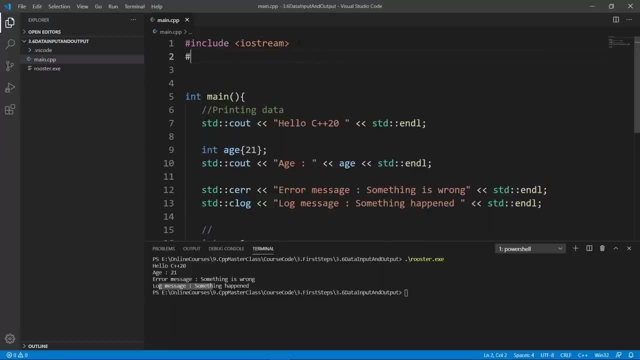 program to store strengths. the way we're going to do that, we're going to include string. this is how you do it in C++. we haven't really learned about this type. it's a powerful type in C++, but we will get to this in the next video. Thank you. 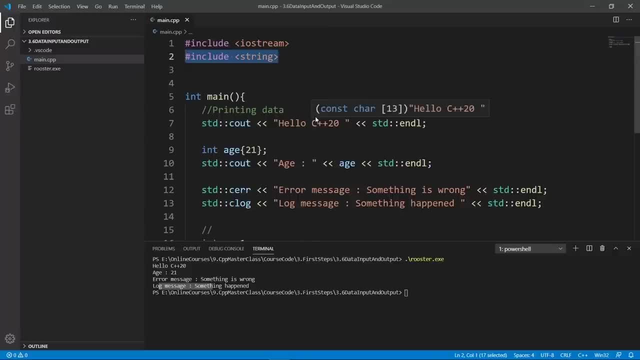 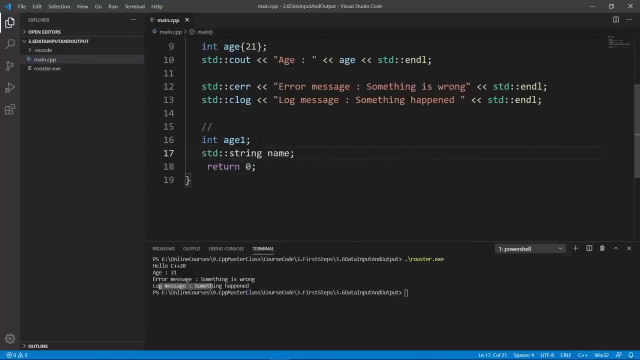 when we have more powerful tools to really understand it. we are just getting started here. so what we're going to do, we're going to say std string and we're going to say name and we're going to ask the user to print their name and age. you, 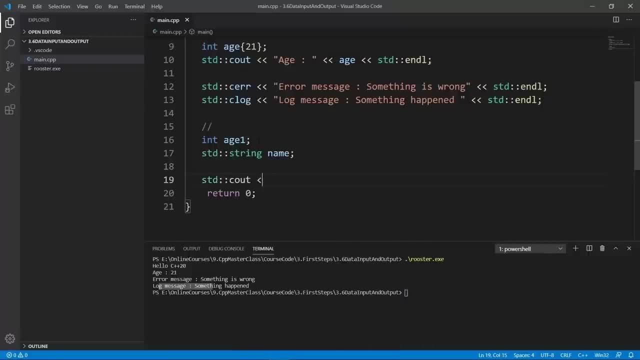 already know how to do that. so we're going to say please type your name and age and we're going to do std ndl on this and how we're going to get data in the program. we're going to use std cin and we're going to do std cin and data is going to be going from the stream to the program. 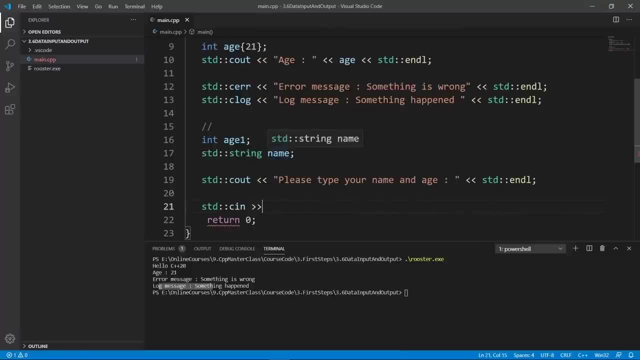 so the stream input operator here points to the right and the data is going to be going in the name variable, because that's what they're going to be typing in first, because that's what we told them to do. so we're going to store the name and we're going to say std cin. that is going to be flowing from std cin into our 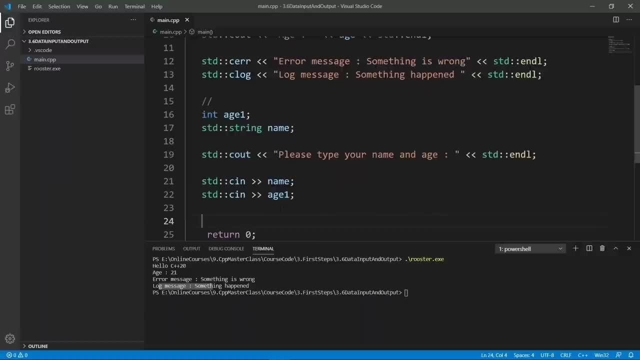 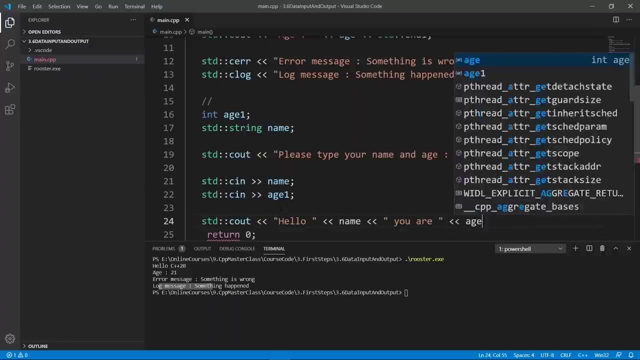 age one variable. okay, now that the user has given us their information, we can greet them with a personalized message. we're going to say std cout, hello. and we're going to put out their name and we're going to tell them: you are, and we're going to put the age one because that's what they're going to give us. 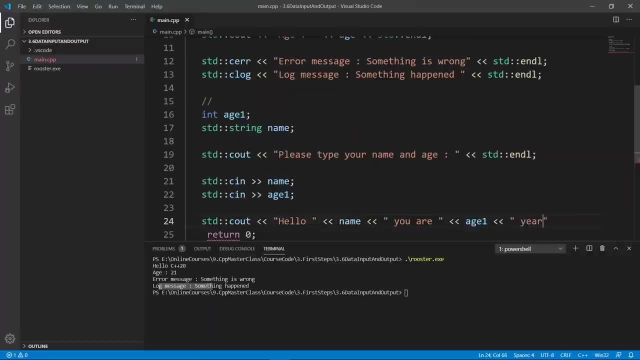 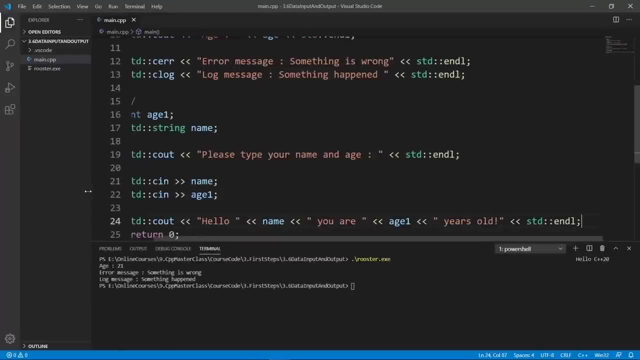 here and we're going to say years and we're going to put an std endl here. I'm going to grab this and pull this to the left and we're going to put the age one left so that we can see our entire program here. that's helpful. so what we? 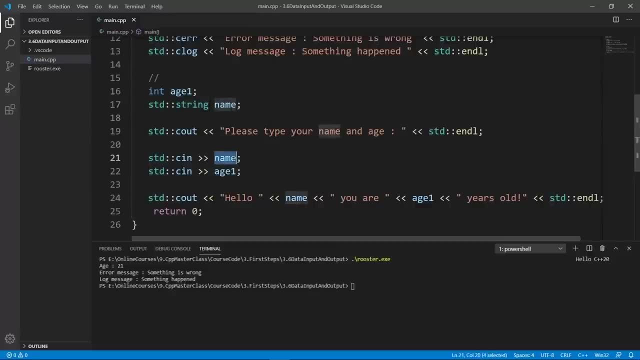 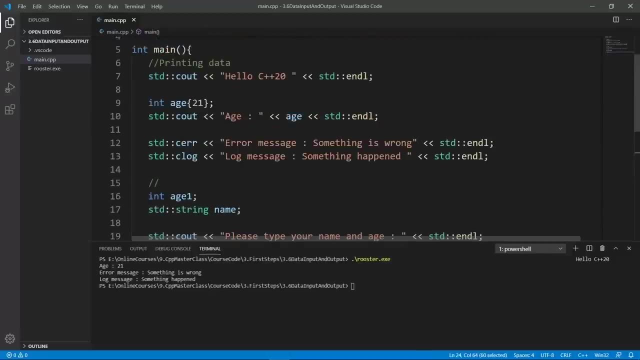 are doing here. we are getting data from the user and we are storing that in our variables and we are printing the message so that the user can see it. I don't want the first things we did here to disturb us when we build and try this out. so I am going to comment this out and comment the first block of code out. 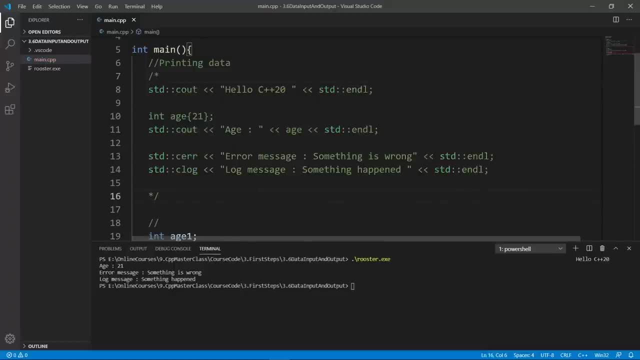 using block comments. I think this is the first time we use this and, uh, this is going to be ignored by the compiler now and it is only going to consider this, and this is going to be pretty cool. let's go down a little bit here and I try to build the. 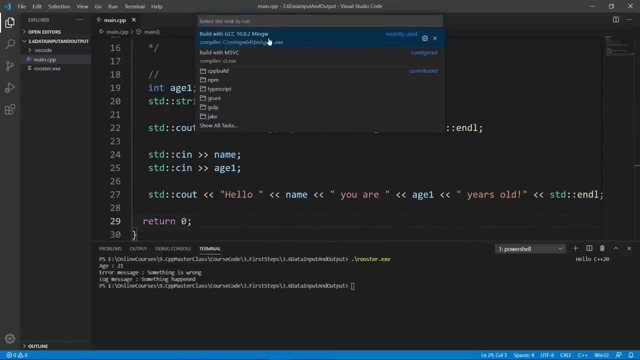 program. we're going to run the task that welds with GCC and looks like the world is good. we're going to hit enter and we're going to clear so that we are not disturbed by this. we're going to run the program. let's say rooster dot exe. it's 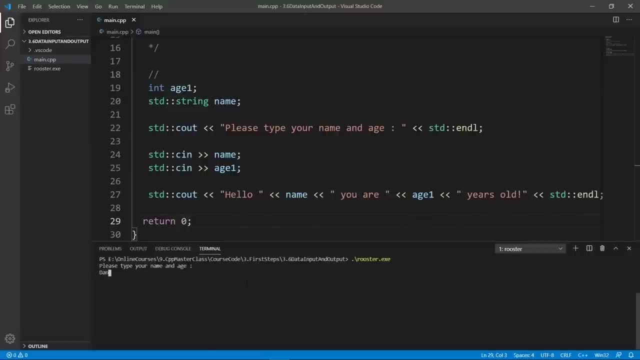 going to ask me to type my name and age. my name is Daniel. I'm going to type that, hit enter. it's going to want me to type my age, so I am going to say 33, for example, and it's going to tell me: hello, Daniel, you are 33 years old. I put a. 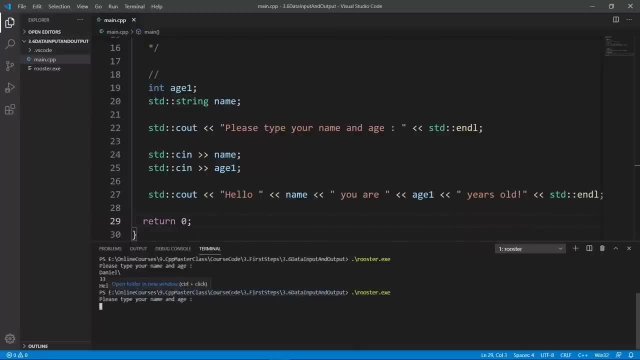 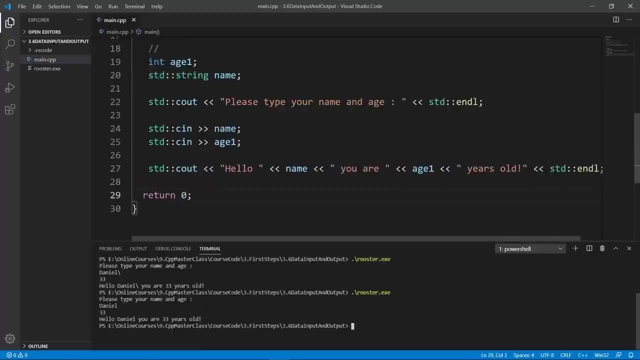 slash here we can try and run it again so that I don't have to make that mistake again. so, Daniel, that's my name, I hit enter, I say 33 and if I run it's going to say: hello, Daniel, you are 33 years old. I really hope this brings the point home that STD CI n is a highway, that. 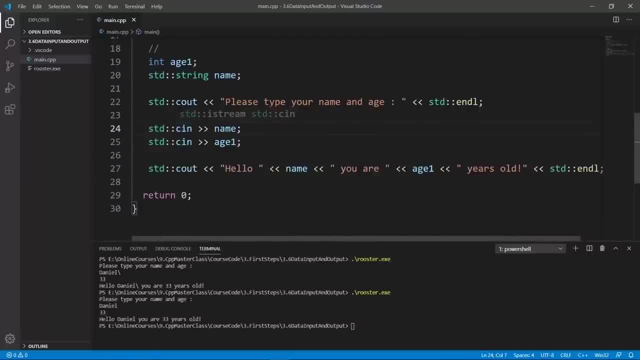 takes data from the terminal into your program. so this is really what is happening here: when I type Daniel, it's going to flow from the terminal and it's going to go into my variable, which is named here. and when I type the age, it's going to go in my edge variable here. and all these happening through STD CI in. 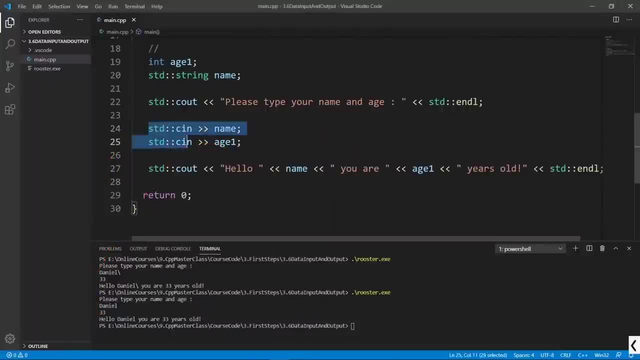 here. okay, one other thing we can do is grab the data and put that in our variables in one go. so what we can do here is comment this out and we're going to do STD CI, n and we're going to put that in name, and we're going to change these two things and put the other piece. 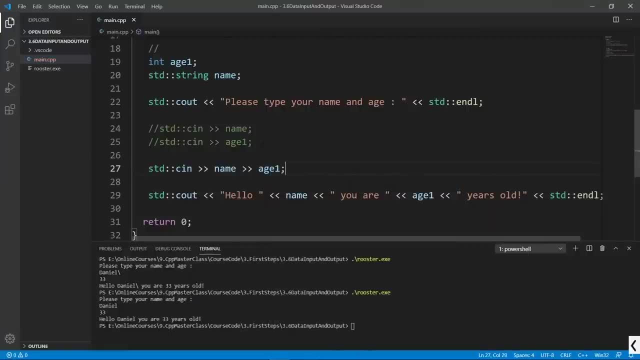 of data in h1. if you run the program, it's going to work exactly the same way, but we are grabbing the data in one line. so let's world to see this in action. we're going to run the task that worlds with CC. we're going to click here and going to clear. if we run rooster, it's going to. 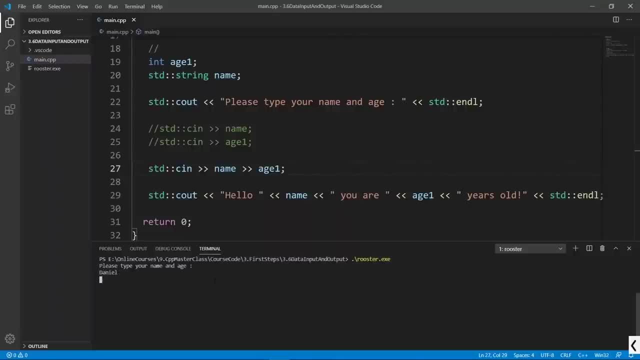 ask for the name and the age. I'm going to put in Daniel, and I'm going to put my age and say 33, for example, and it's going to do exactly the same thing, but we have one compact line. the last thing I want to show you in this lecture is: 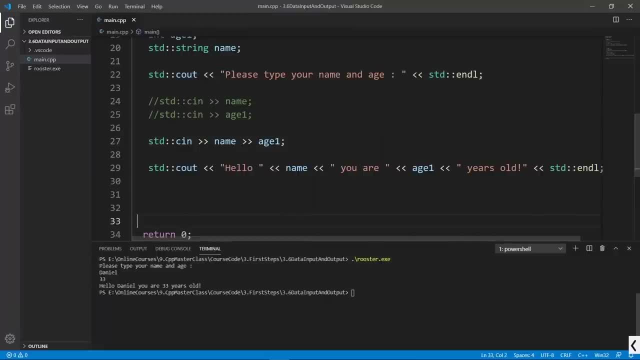 how you can grab data with spaces, because if I try to put in data with spaces here, the program is going to fail miserably. let me show you this. I'm going to clear and I'm going to run rooster again and I'm going to say: Daniel, I'm going to put in my full name and it's. 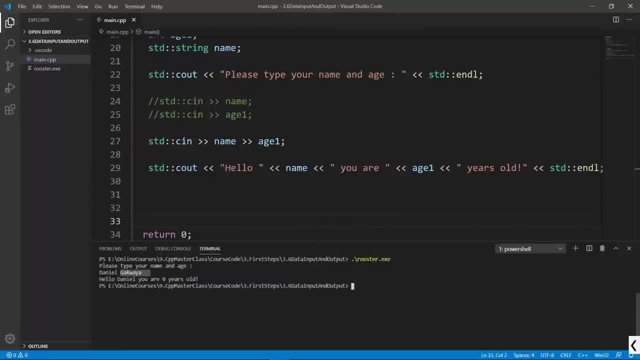 really not grabbing the second name, and it didn't give me a chance to input my age, and this is really bad. so C++ provides a way to solve this using STD get line. so let's say what we are doing here and before we play with this, 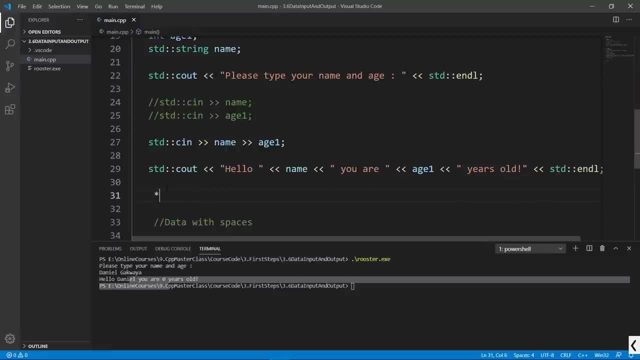 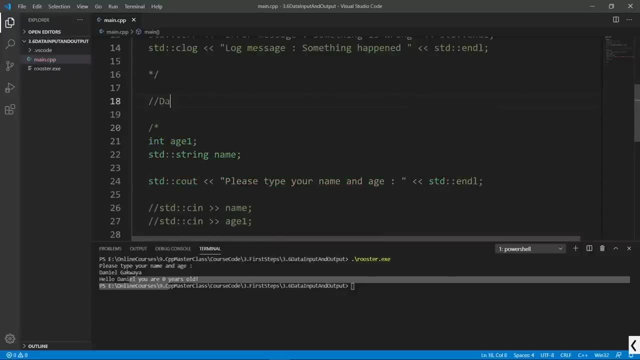 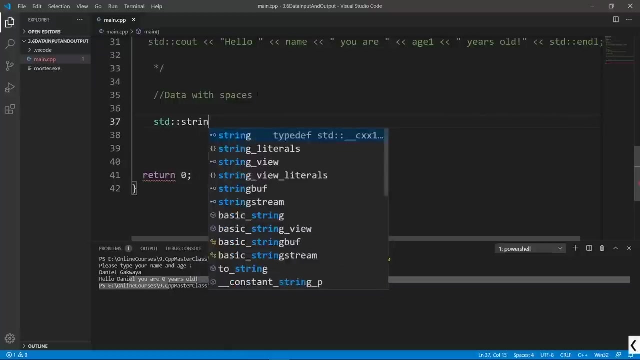 we're going to comment out what we had here so that it doesn't disturb us in what we are about to do. so let's come down here. we were doing data input- this is helpful here- and we're going to go down and grab data with spaces. so I am going to set up another strand and this is going to 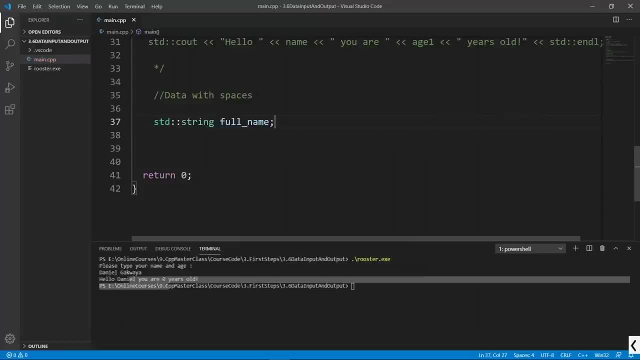 store my full name. that's what I'm going to say here- and to grab it, I'm going to tell the user to type in their full name and age. so I am going to STD, see out. so the way I'm going to grab the data, I'm going to do STD, get line. you see that we. 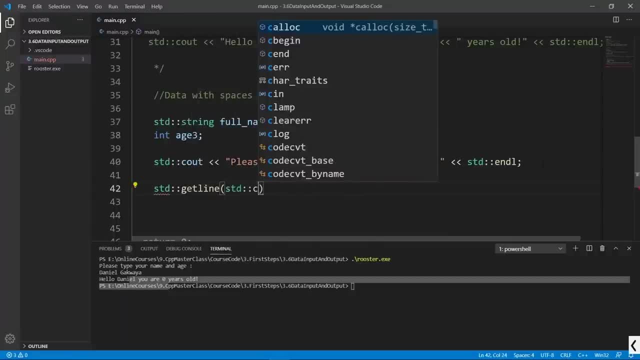 have this function here and it's going to take an input stream. so a STD- see I'm in- is going to work, and the second parameter is going to be the variable where this string data is going to be stored. we're going to pass in our full. 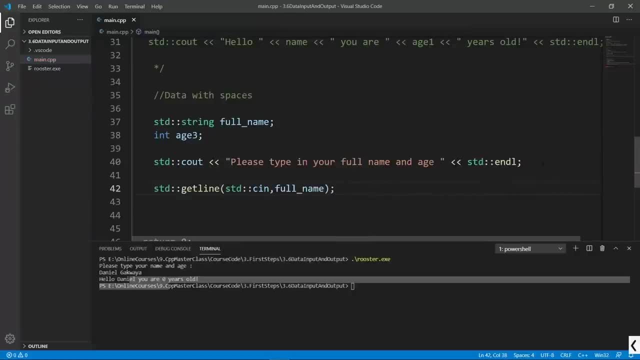 name and this is going to work just fine. and we're going to also grab the age using the same technique we've used before. so we're going to say STD, see, I am, and we're going to store that in our age three variable. once we have the data, we 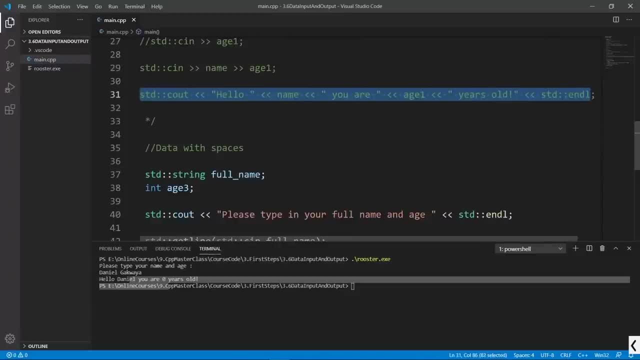 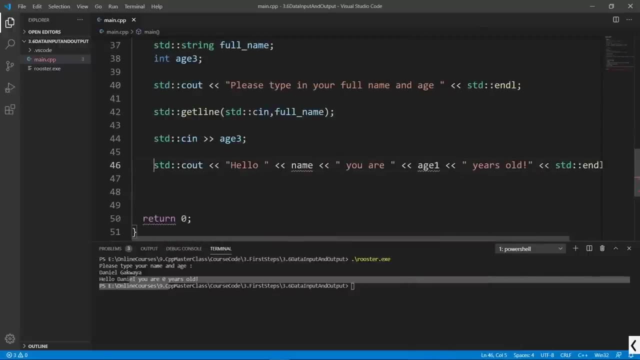 can greet our user using the same message we had before. so I'm going to copy that, if I can do that, and then I'm going to copy that, and then I'm going to paste that here. I'm going to bring this to the same location it's going to be. 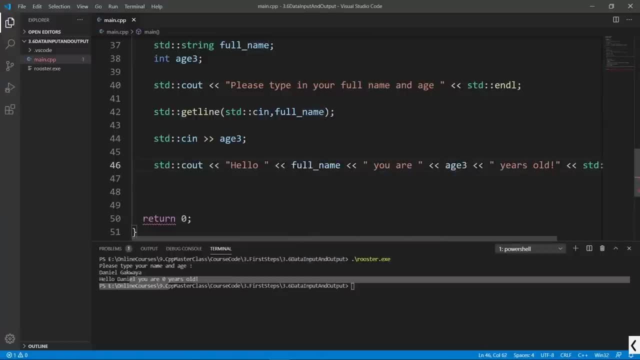 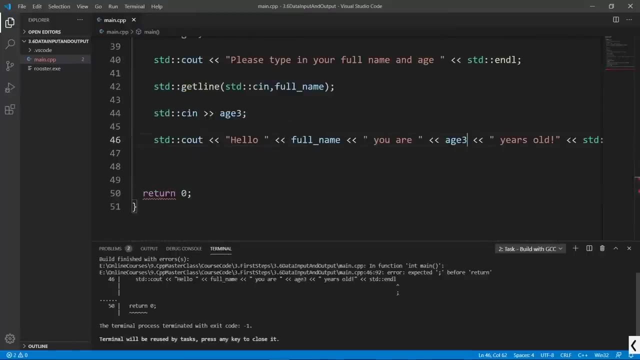 full name here and it's going to say age three and let's try and world. we're going to terminal, run the test world with GCC and we have a problem because we forgot our semicolon. see how these problems might come to you, uh-huh. so we're going to put in our semicolon. and another thing I really 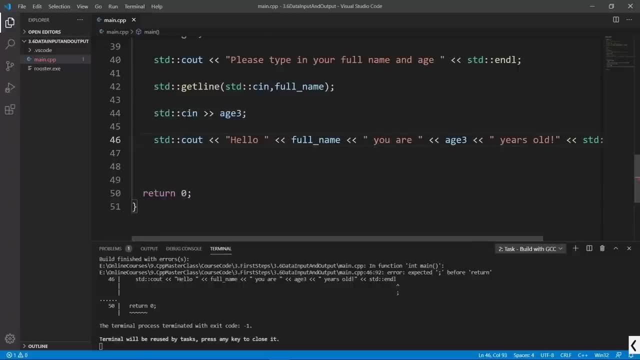 want you to see is that you can bring these things to the next line if they turn out too long, like we see here. so I can, for example, put this to the next line, and it is going to work just fine. so what I am going to do, I'm going to 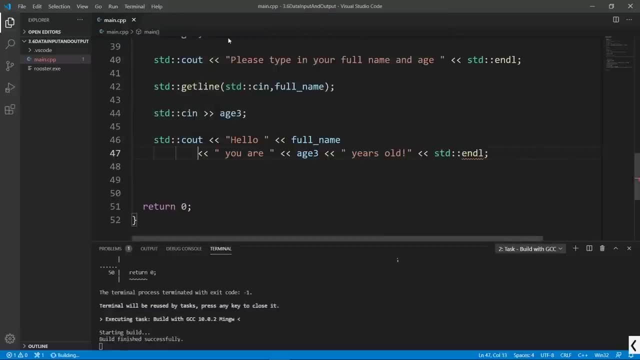 try and build again. run task to world with GCC- you see that the world is good- going to bring in our terminal. I'm going to clear so that we don't have noise here and we're going to run our program. it's going to ask me to put in my full name. 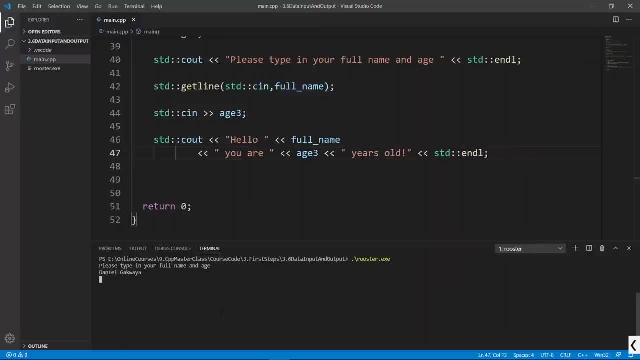 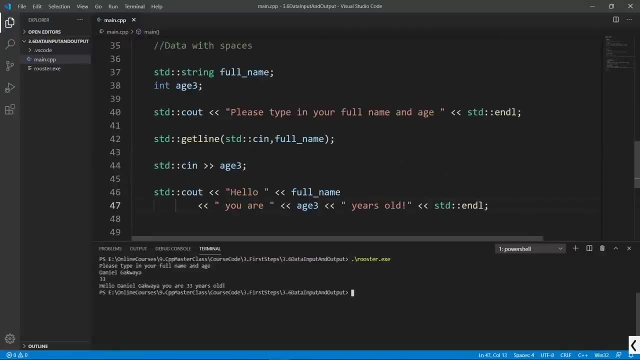 I'm going to say Daniel cap wire, and it's going to want the age. I'm going to say and it's going to reach me: hello, Daniel capoia, you are 33 years old. we are able to bring data with spaces into our program and this concludes what we had. 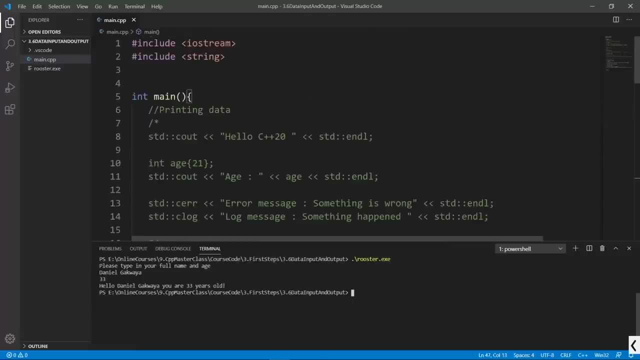 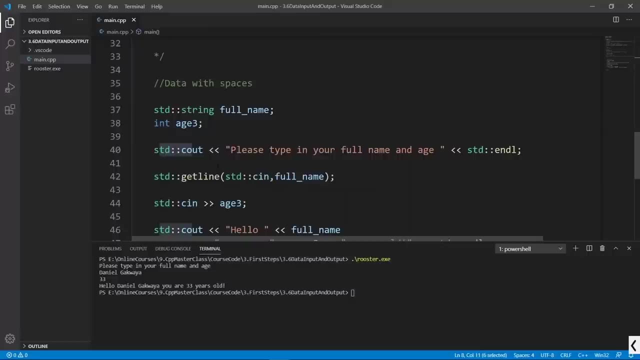 to say in this lecture. I hope it made it very clear what these stdn and stdc out things are. they are basically highways that take data out of your program or bring data into your program, and the way you use them is what we've done here in. 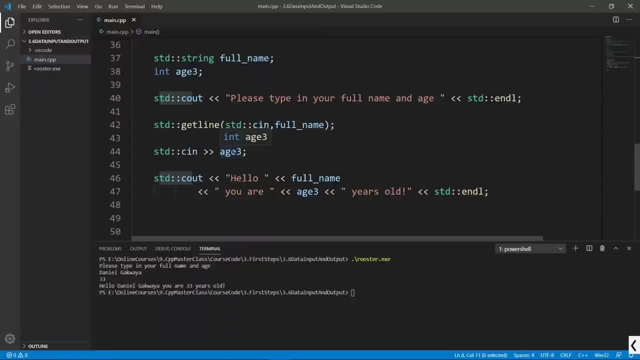 this course. I would encourage you to play with us a couple of times. if this is the first time you're doing this, we are going to stop here in this lecture. in the next one we're going to try and recap on the C++ development workflow. go ahead and finish up here and meet me there. in this lecture we're going. 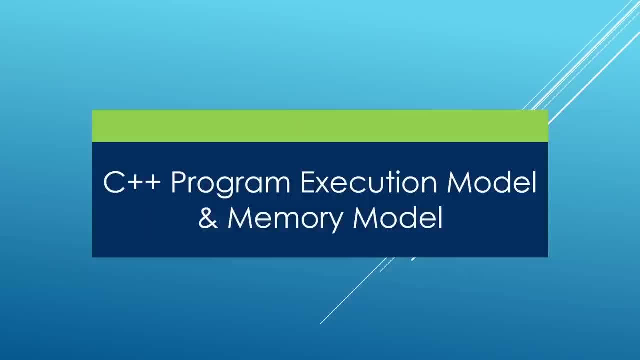 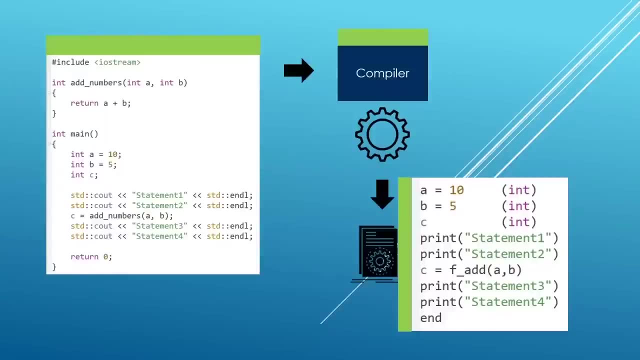 to explore the C++ execution model and show you a simplified version of the memory model of your C++ program. here is how our program looks. it is a simple program. in our main function it is going to call a paper function that is going to add two numbers. we have seen a program like: 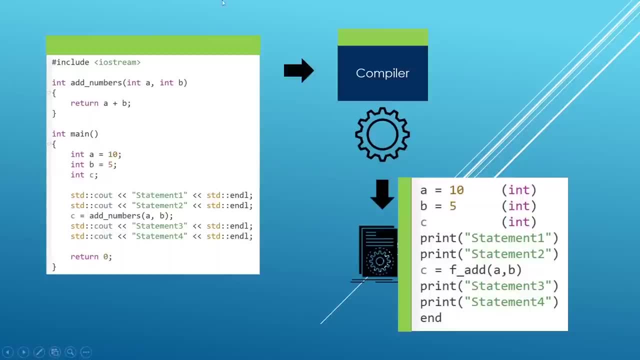 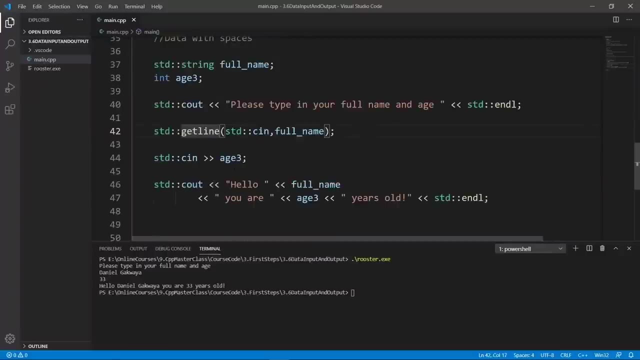 this before and when we compile it. it's going to be turned into a binary. this black icon here represent the binary executable and it is not in the format that you can read with your eyes. if we come back here to what we were doing in the last lecture, we can see our rooster executable binary here if we try to open. 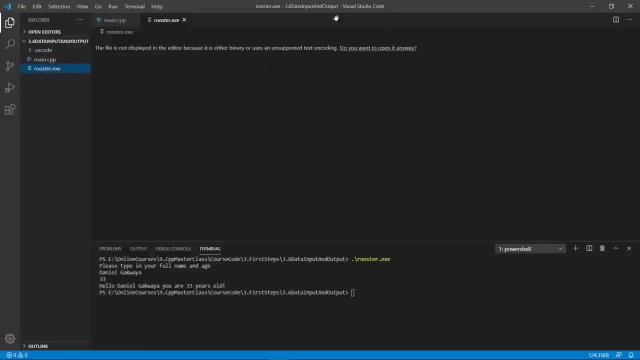 it here. you're going to see that visual studio code is going to say: the file is not displayed in the editor because it is either binary or uses an unsupported text encoding. so it says: I can't really say this, because it's binary and it says: do. 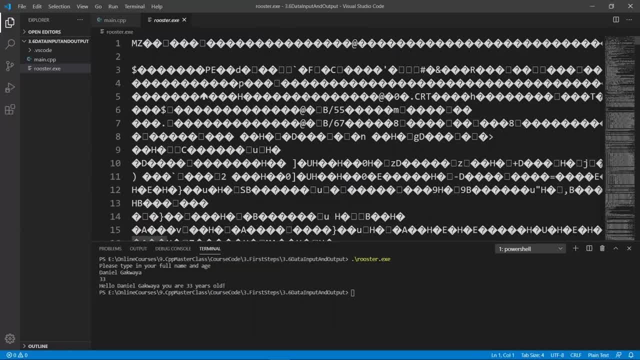 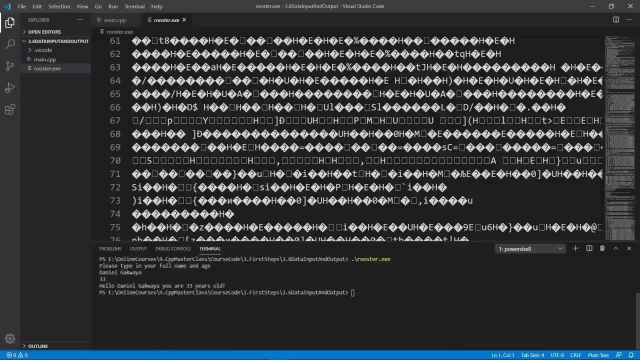 you want to open it. anyway, if I try to open it, it's going to be just some gibberish, because this is binary. it is meant to be read by programs. it is not meant to be by IDs or text editors like Visual Studio code. so this is the binary. 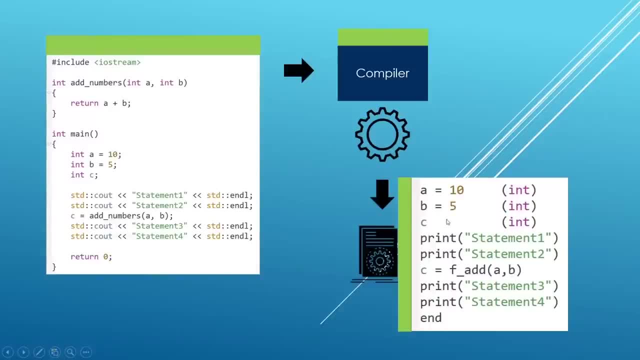 file we have here. I tried to put a simplified version of this program to represent binary so that we can follow it up, but it is not in the form that is readable by any human out there, unless you are a machine. so why is it in binary? because binary format is easily understandable by 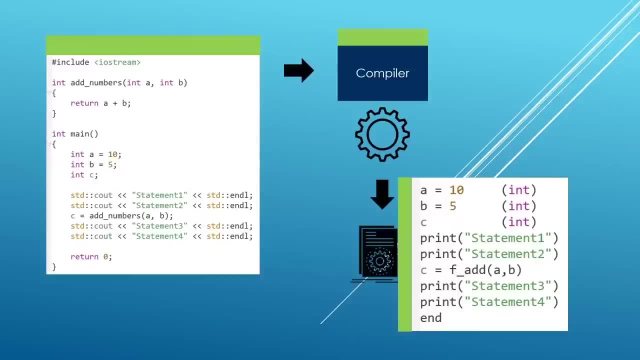 your CPU and we're going to see how your program is loaded in memory and executed statement by statement by the CPU, so that you can really understand this. so here is a representation of your program. here we have our hard drive and we're going to see how it is going to look like in the next video. 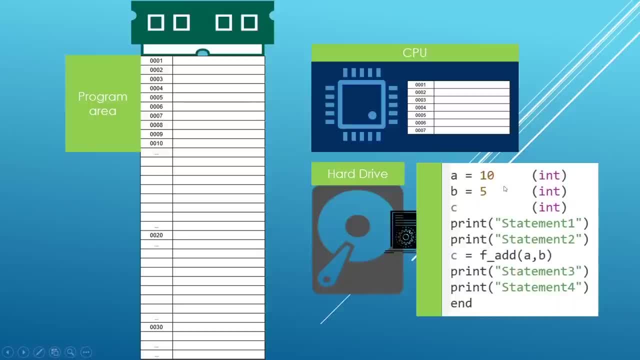 we have the program sitting somewhere on our hard drive in binary format and it's waiting to be run by you by double clicking on it or opening it in the terminal. and on the left here we see a representation of the memory of our computer. and when I say memory, I mean random access memory. I don't mean memory. 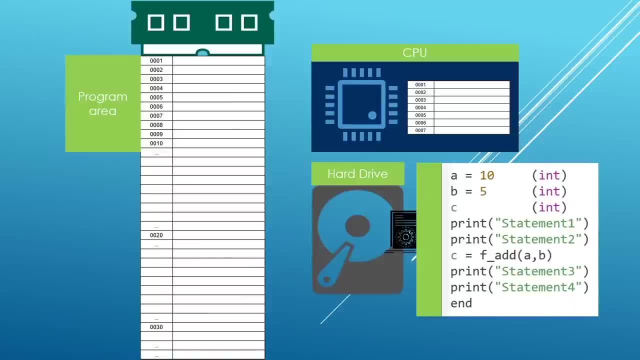 on your hard drive. this should be really clear. this is the random access memory of your computer that is running your programs very fast. so when you double click on our program or if we open it in the terminal, the binary file is going to be loaded up in memory and you see it in red here. this is a representation of that, and it is. 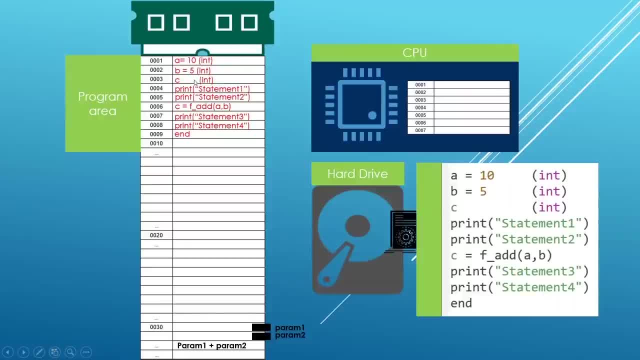 ready to be run by the CPU. by the time the CPU sees in the memory location, it's going to know I have a program to run and the CPU is going to start running it statement by statement. it is going to start by the top, so it's going to see that it needs to allocate space to store our 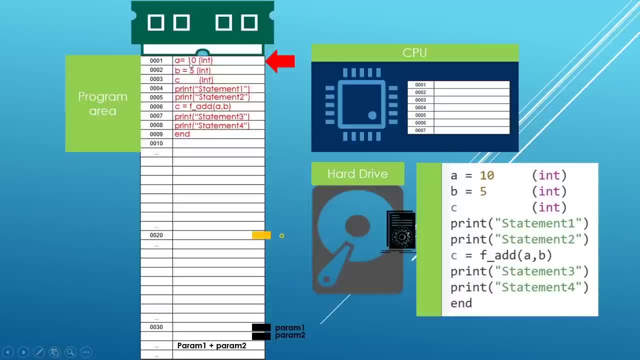 integer a. it's going to allocate to that somewhere on the memory. in yellow here you see a and it's going to see that it should store in a value of 10 and it's going to do that. you can see that here. it's going to go to the next statement and the next statement tells it to: 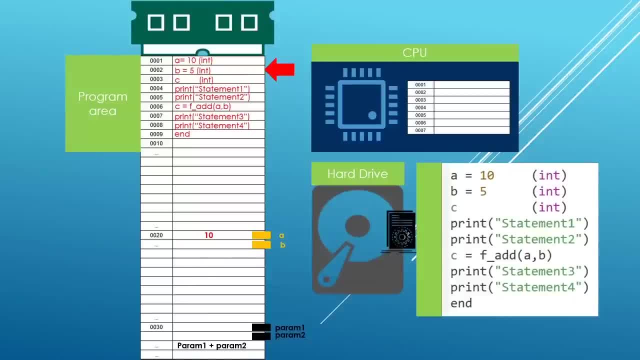 allocate space for a value B and it's going to store in a five. it's going to go to the next statement. it's a variable called C. it's going to allocate space for it, but we didn't specify a value B, so what it's going to do is store in some junk value. the value in there is really unspecified at. 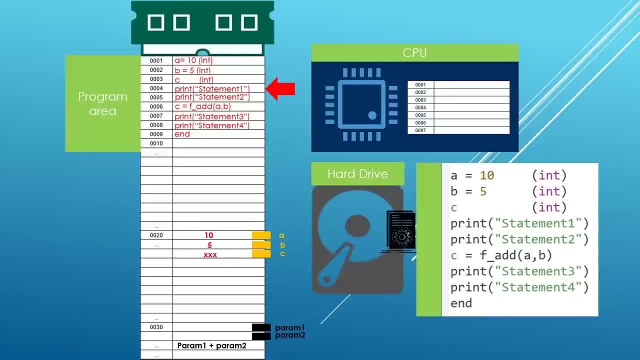 the moment it's going to jump to the next statement and what it's going to do is print some things on the console. and it is going to do that. it's going to jump to the next statement and it is going to print statement too, and here it is going to notice that it is going to call a function I don't know. 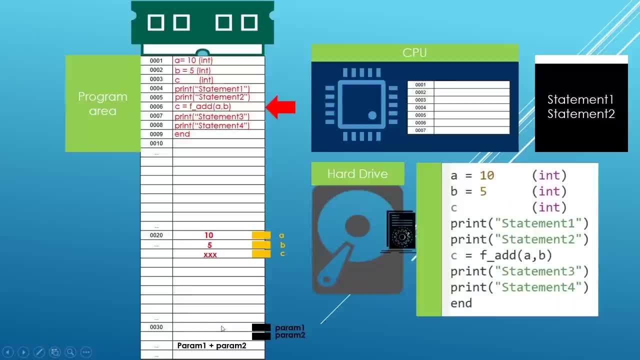 if you have noticed, but the CPU has allocated a special memory location for our function. the function doesn't leave with our code here or anywhere near the variables that we have here. there might be a huge chunk of memory between these two or three things, so the CPU knows that. 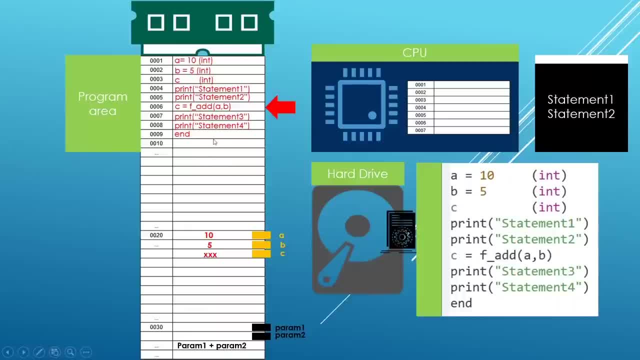 it is going to jump to another location. it's going to ask itself: if I jump to that location to run this function, how am I going to come back? and the CPU is smart enough to store the return address. and that's what it's going to do. it's going to say: if I go to that function, I want to. 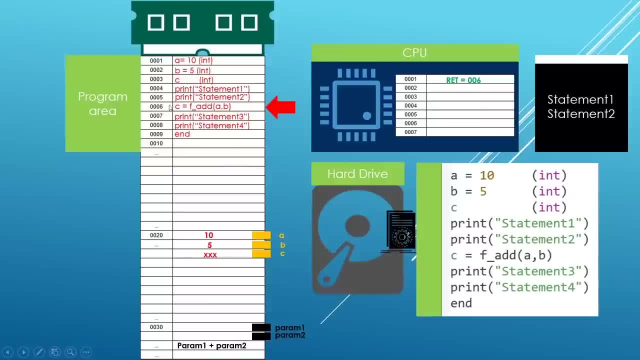 come back to the address 6 and run whatever is after this address. so it's going to store six and CPU memory and it's going to jump to the function. it's going to take the first parameter as a and the second parameter as B. so a is 10, the parameter one is going to be 10.. it's going to take parameter two. 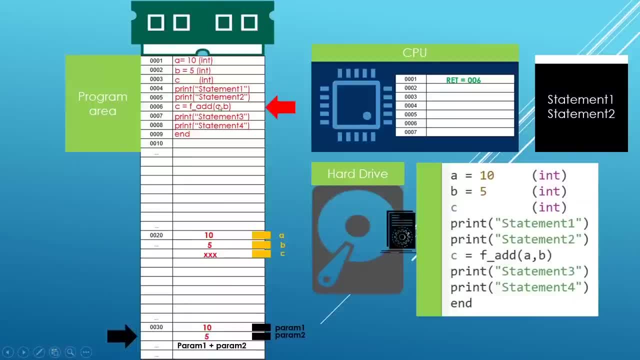 it's going to be five, because it is B here and in B we have a five, and it is going to jump to the next statement in the function and it is going to add up parameter one and parameter two. after it adds those things up, it's going to return the result to C. we can see that here. okay, that's what. 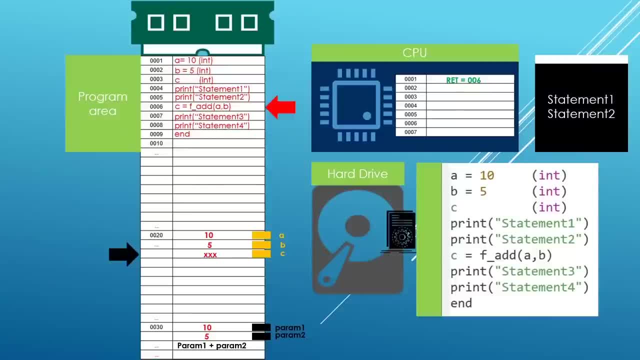 the CPU is going to do. it's going to put the result in C and the result is a 15, so we're going to write that in there and now that the function is really done, it's going to come back to its address and it is going to jump through the next segment. after that, it is going to print three. 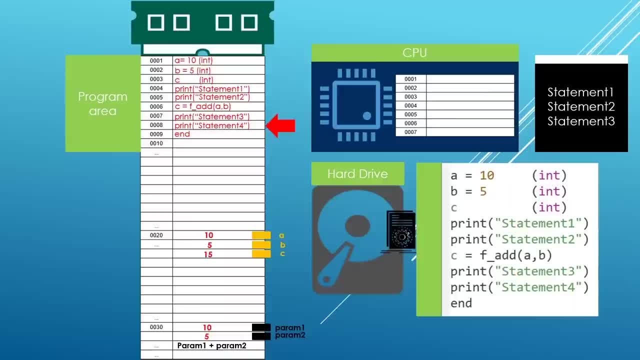 statement three. it is going to jump through the next line and print statement four. it's going to do that and by this time we have reached the end of our program and it is going to be popped off the memory and your program is basically going to end. this is how your program is executed by your CPU. 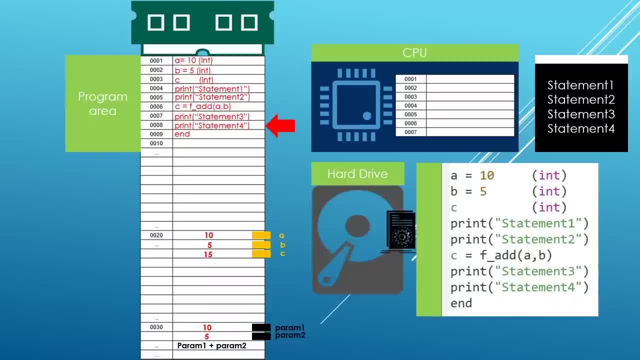 and why am I showing you this? because it is really good to have an idea of how memory is allocated and used by your program. another good reason is that some C++ feature require you to have an understanding of a memory model like this to understand how they work. 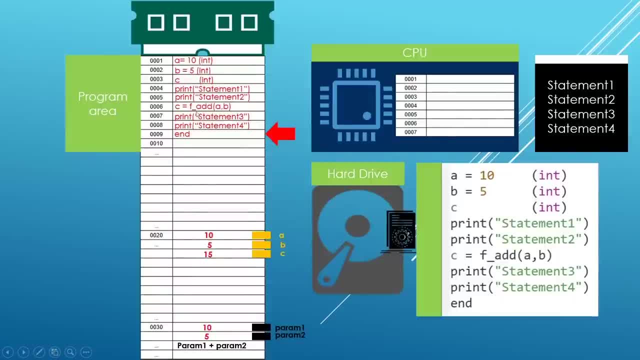 for example, you have seen that to call this function the program had to jump from address 6 to 30. and this is really heavy, especially if you are running a simple function, like we are doing here, to add two numbers so the CPU can realize that and optimize this call to the. 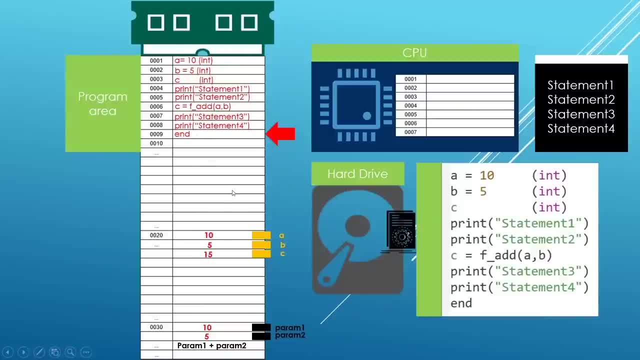 function to an inline function and add these two numbers up right here at address sex, without jumping to this address here, and this may come in handy, and you need an understanding of this memory model to really understand these features. this is just one example I am giving you. you are going to 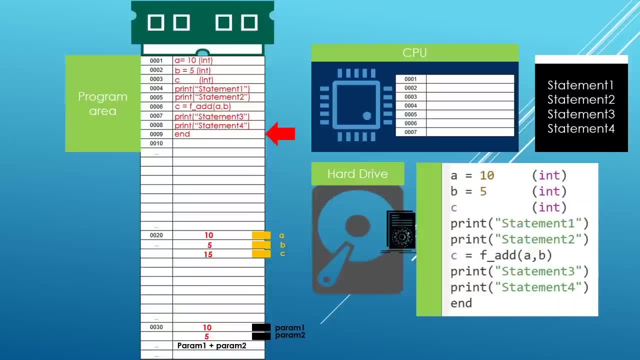 reuse this model a lot in your career as a C++ developer and I thought it was a really good idea for you to understand it firsthand. this is really all I had to share in this lecture. I hope you found it interesting. in the next one, we're going to try and understand the difference between three key. 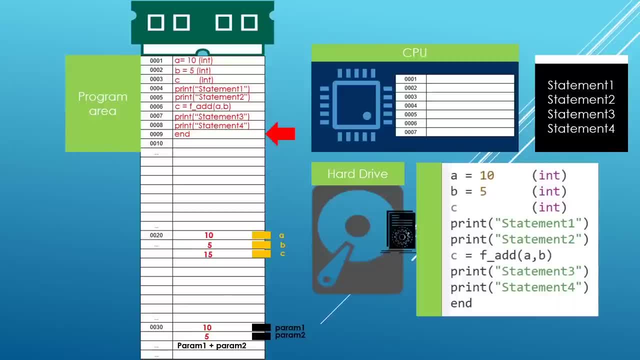 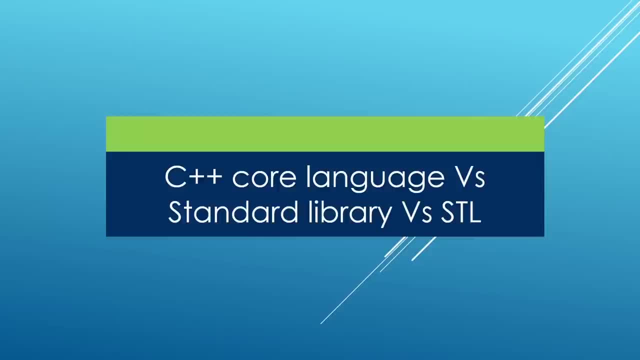 components of the C++ programming language. go ahead and finish up here and meet me there. in this lecture, I want to highlight the differences between what we call a C++ core language feature or a standard library feature or an STL feature, because these are terms that come up a lot. if you happen to read some 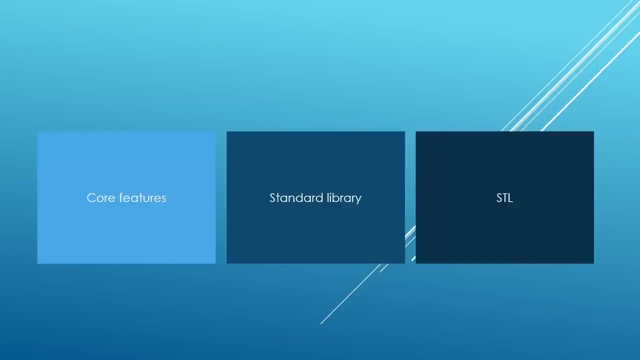 documentation about C++. a core feature is really a basic welding block that makes up the C++ programming language. you can think of it for example, how you define variables, the rules that govern how you can define and use a function in C++, the rules that say what you can do and not do with the basic features of C++. that's 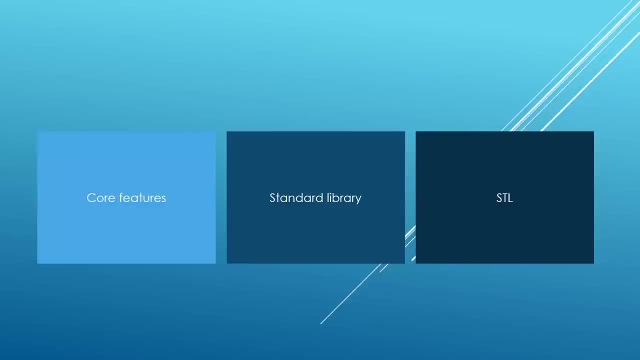 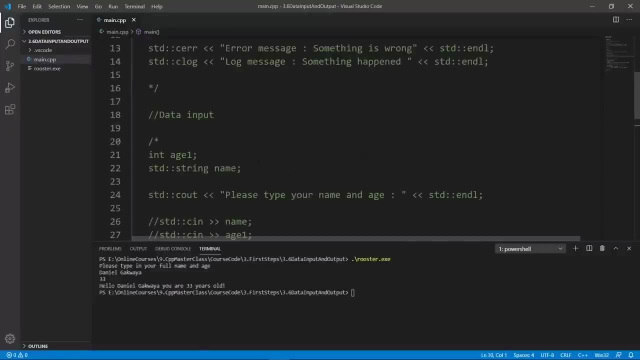 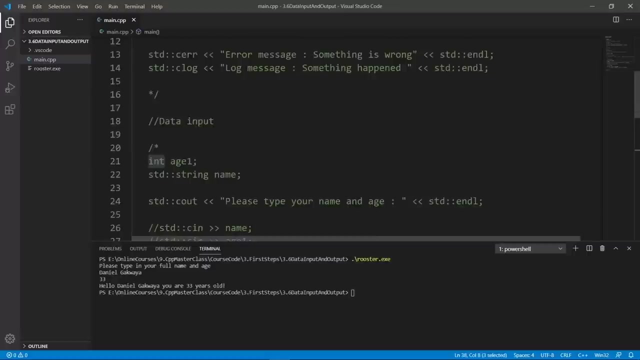 really what can be qualified as a core feature of the C++ programming language. I don't know if that makes any sense. if we come back in Visual Studio code, we have a program we have used in the last few lectures, for example, these basic types that you use in C++, the rules that define how you can. 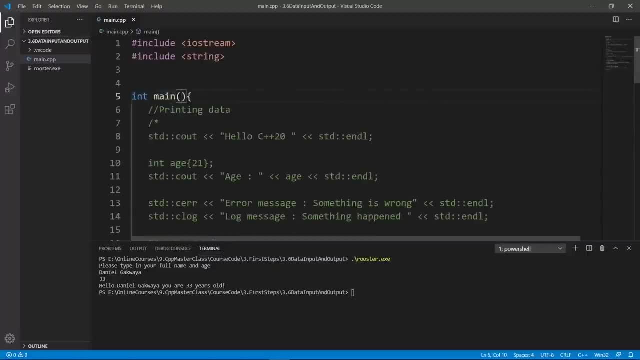 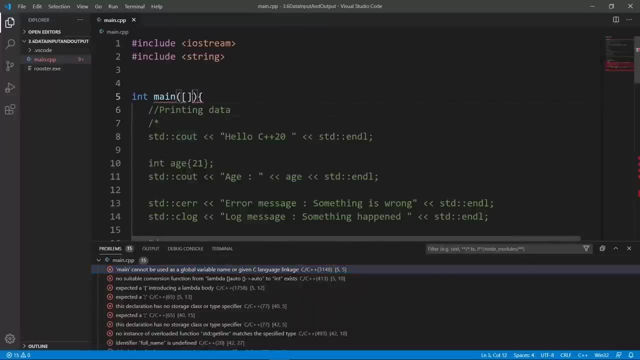 define a function. for example, if you put a nanobracket here and try to compile this program, it is not going to work because we have violated the rules of the C++ programs, the basic rules that define how the C++ programming language works, the basic types that are defined in the C++ programming language. this little thing. 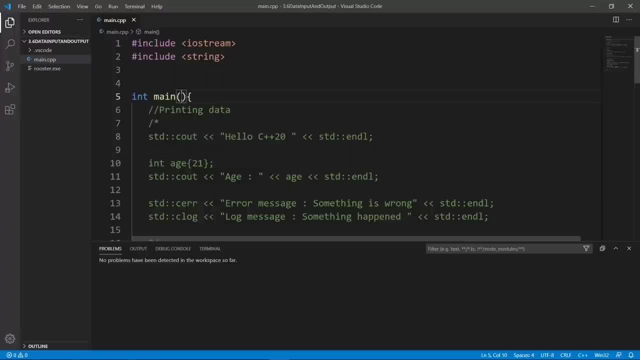 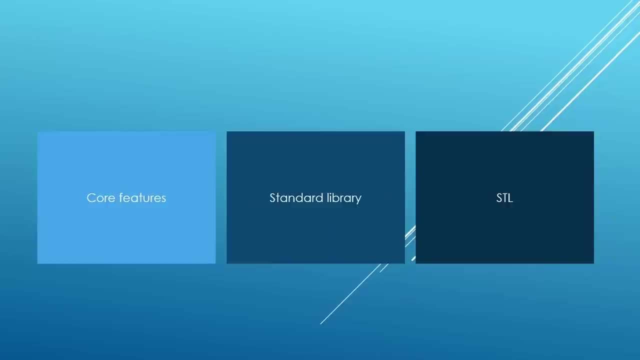 to make up the row ingredients you use to make up a proper C++ programs, and these little row components you use to put together a c plus plus program are called core features. you can think of them as the foundation on top of which we really build. daily use c plus plus programs, the standard. 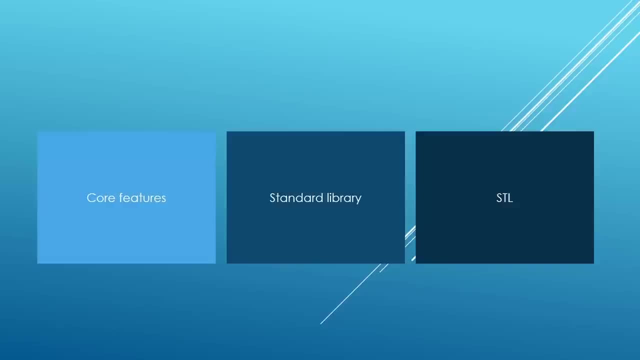 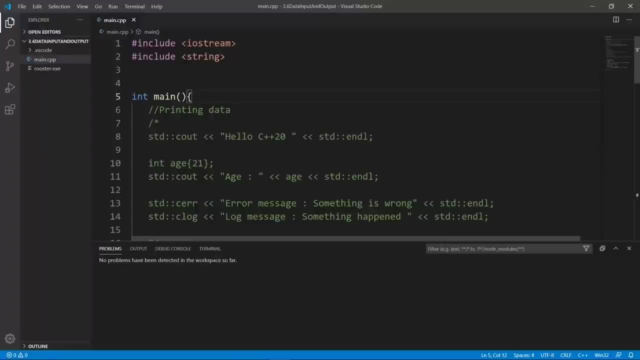 library is a set of ready to use highly specialized components that we can easily use in our c plus plus programs. and again coming back to our program, in visual studio code io stream, here is a standard library feature string. here is a standard library thing we have in the c plus plus programming. 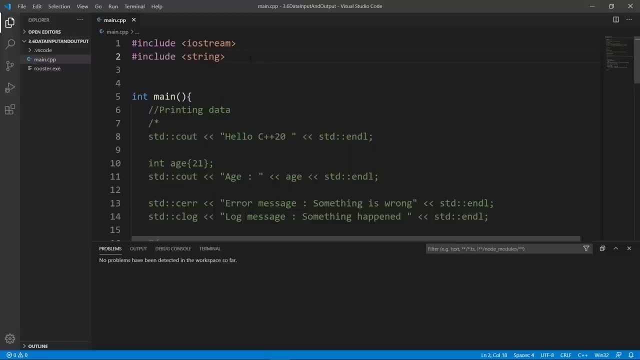 language. and again, the c plus plus standard library tries to provide highly specialized components that we can use in regular c plus plus programs. when you use the c plus plus programming language, you don't really want to extend the c plus plus programming language you want to use. 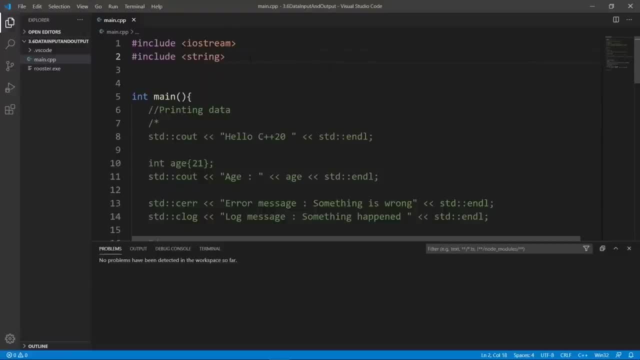 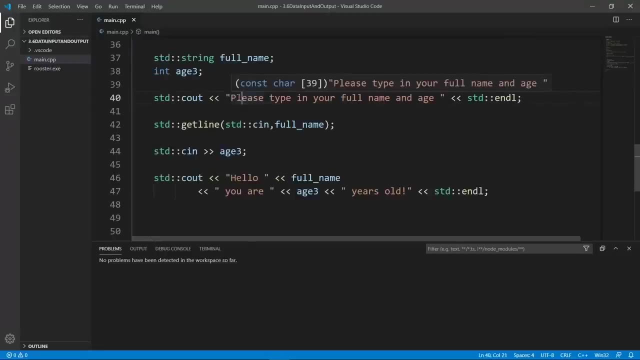 it to build something of your own. and, uh, the standard library feature is the c plus plus standard library and the standard library is the c plus plus standard library. for example, we have used stdc out without really going into the details of how the data is taken. 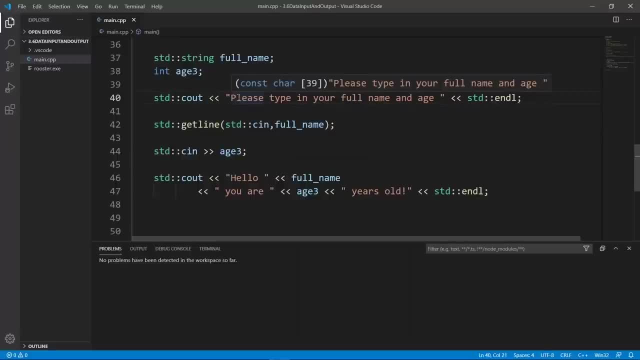 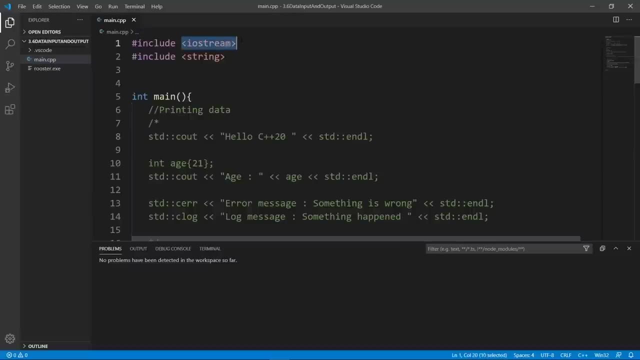 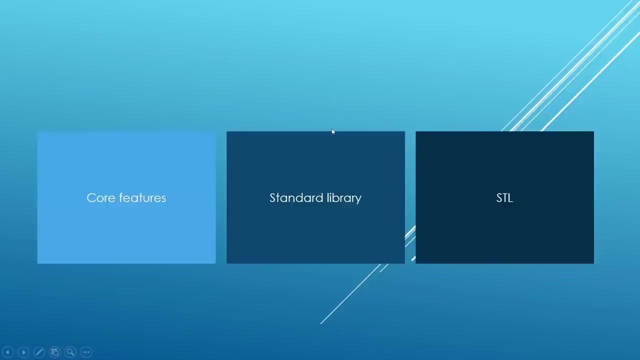 from this program to the terminal. that's really advanced and probably complicated, but it is wrapped into this reusable components and one of them is io stream and we can use it relatively easily in our c plus plus program. okay, i hope now you have a better idea of what the c plus plus standard. 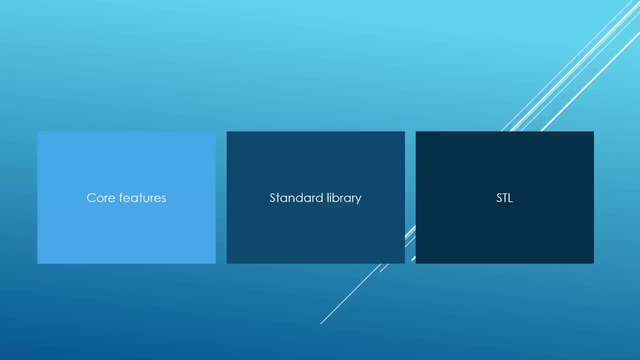 library is. now, what is the stl? the stl is really part of the c plus plus standard library, but it is a collection of container types. think of them as collections of things, and we have a set of types that allow us to store collections. we have algorithms or functions that work on these. 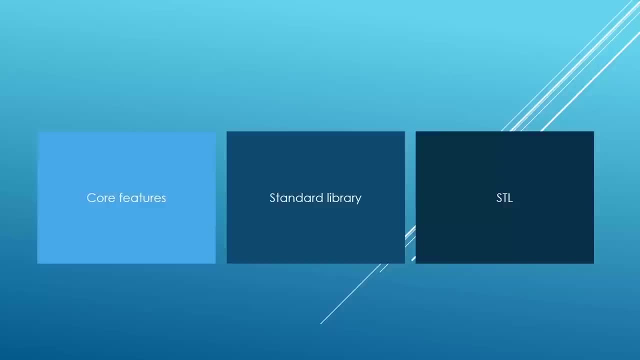 collections and we have specialized types that are called iterators that allow us to navigate through these containers, potentially running these algorithms on each element in the collection. this is probably not making sense by now, but you can think of the stl as a highly specialized part of the c plus plus. 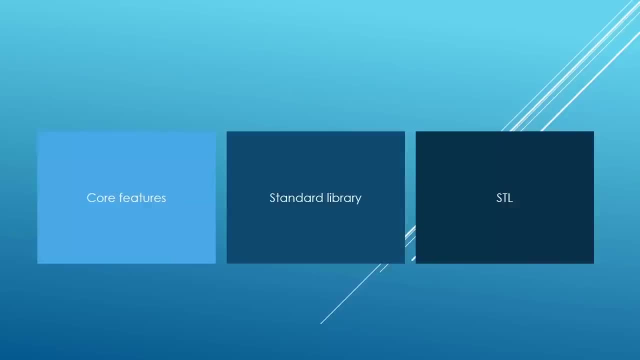 standard library and we're going to learn about many features of these things throughout the course, but i want you to have a basic understanding between these three terms: a core feature of the c plus plus programming language, a standard library feature and the stl, and i really hope this is clear to you by now. in this chapter we're going to learn about variables. 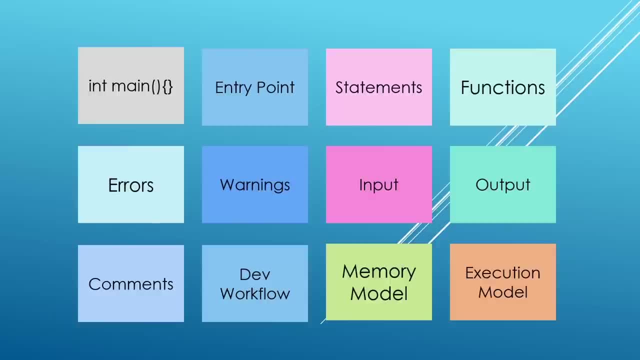 and data types. before we talk about variables and data types, i would like to take a moment and recap on what we know by now, and if you look at these cards, many of these things should make sense now. you know about the main function. you know that it is the entry point of your program. you know that. 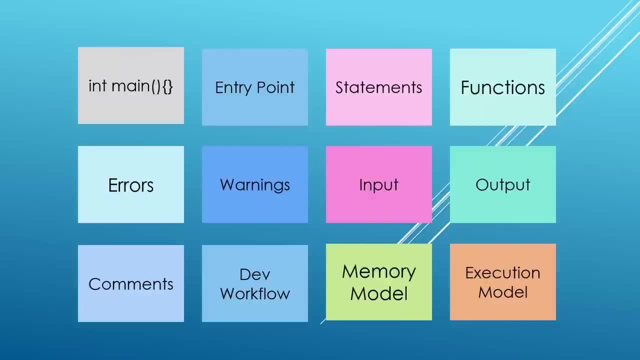 your program is going to be made up of statements and statements and with a semicolon in c, plus plus. you know about functions, errors, warnings. you now have an idea about how you can handle input and output from your program. you can use comments. you know about the memory model and the execution. 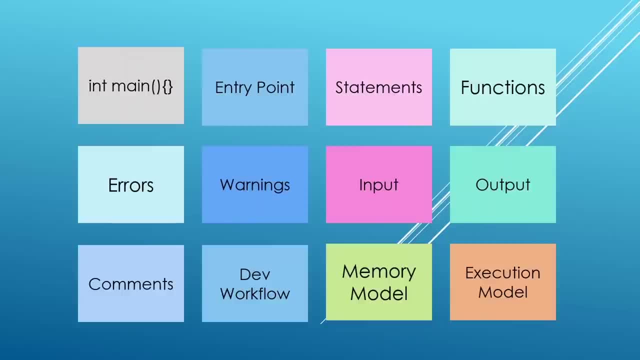 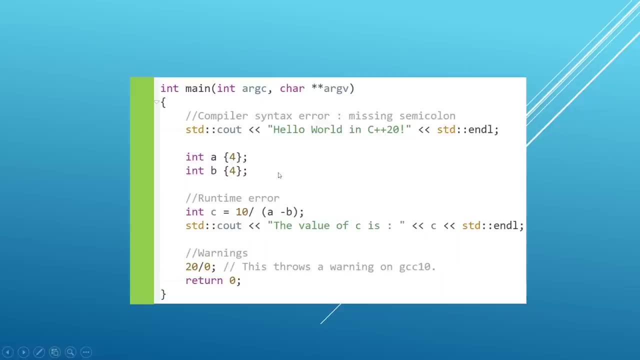 model that we talked about in the last lecture. you know quite a lot now. we have been using a program like this to do things in the last chapter, but there is one thing that isn't really explained yet, and that is this ant. this ant is a type that is predefined in c plus plus. 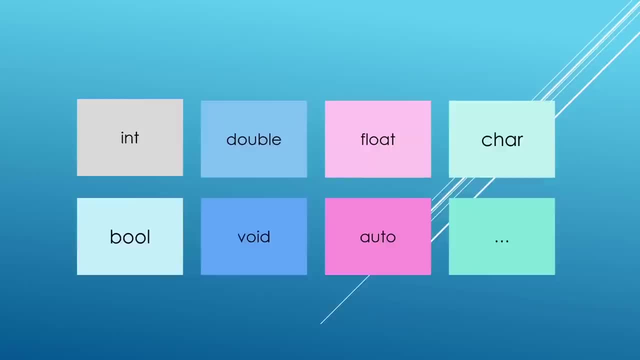 and c plus plus pre-defines many types here. we have a couple of these types for you to see as examples. ant is one of them. we have seen it a lot of times in the last chapter. it is used to represent whole numbers like one, two and three. but we have others, for example, double and float are. 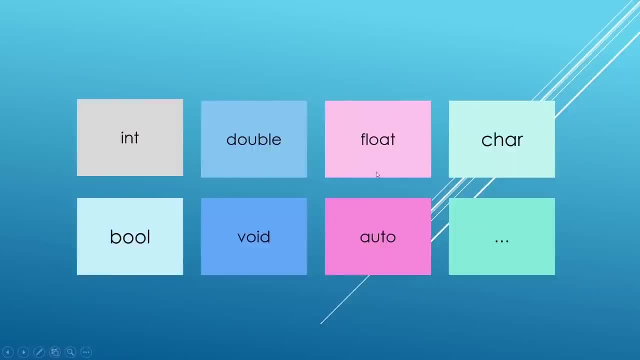 used to represent fractional numbers, numbers that have decimal points- for example, 2.5, 7.3- and numbers, and we're going to see the difference between these two. another one that is commonly used is char or car, and it is used to represent characters in memory and you can store. 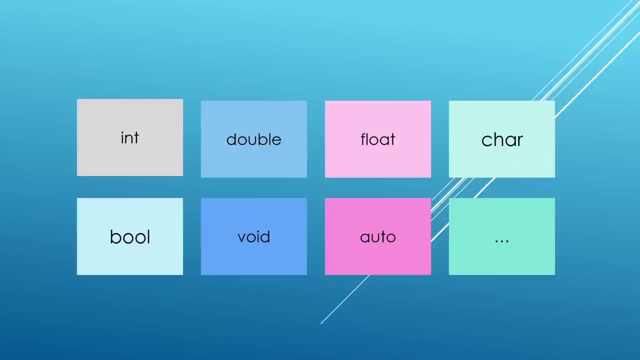 in characters like a, b, c and d and all the other characters you can really put in. we have a bull, which is a type that is going to store two possible states. the only values you can really store in here are true or false, and we're going to see how this works. void is a somewhat. 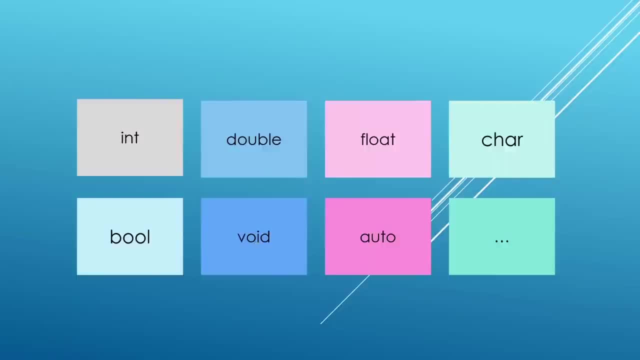 confusing because it represents a typeless type and it is really meaningful when we get to talk about functions in detail. so we're going to learn more about the void type a little later in the course. we also have the auto type, which is really not a type. it is a keyword you use in c plus plus. 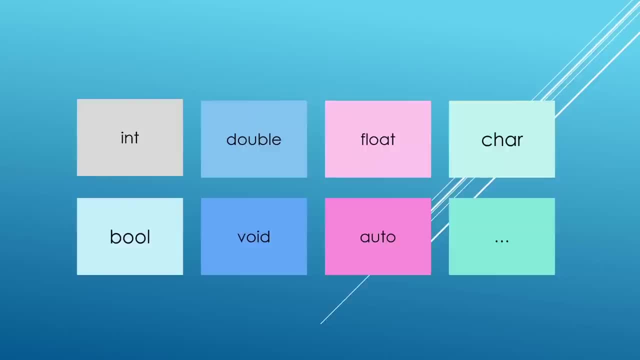 to deduce other types, and we're going to see how this works later in the course. these are a few examples of types we can use in c plus plus, and we are going to play with most of them in this chapter. another thing i really want you to see is what. 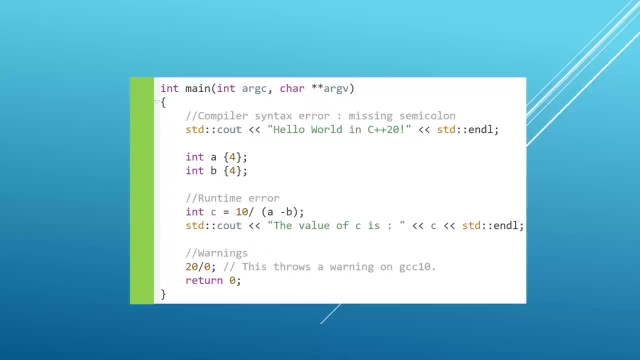 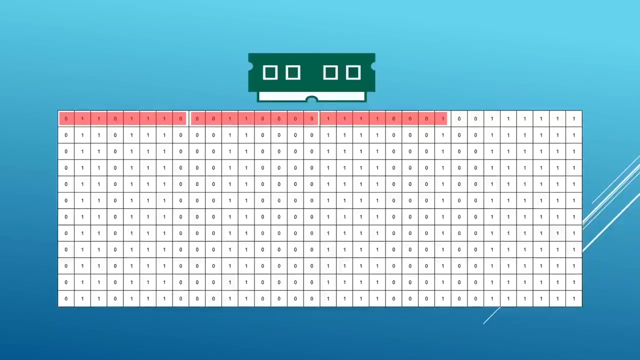 does it mean to really put a four in a variable in your program? everything you have in this program here is represented by ones and zeros in the computer's memory. it really looks like this: it's a bunch of ones and zeros in the ram of your computer and there must be a technique to make. 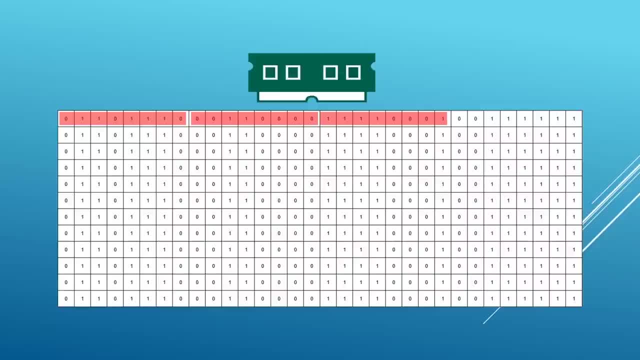 sense of this gibberish here and store data that makes sense to humans. and the starting point is to group these ones and zeros into little chunks that we can manipulate. each of these ones and zeros is called a bit, so this zero here is a bit, this one here is a bet, and if we group eight, 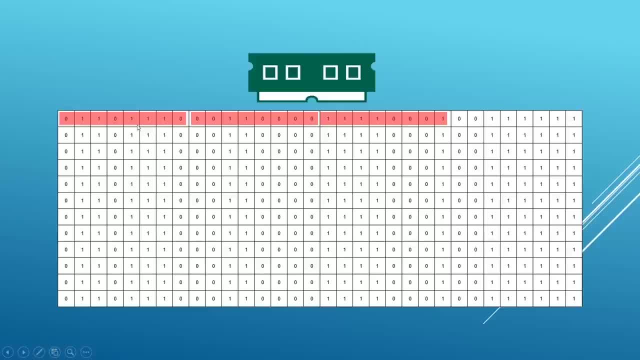 bits together. they are going to form what we call a byte. okay, if it makes sense, you can group your bits in bytes. or if it makes sense to group them in groups of 16, you can do that like we see here. we're going to see a little more details about this in the next lecture. okay, here you see. 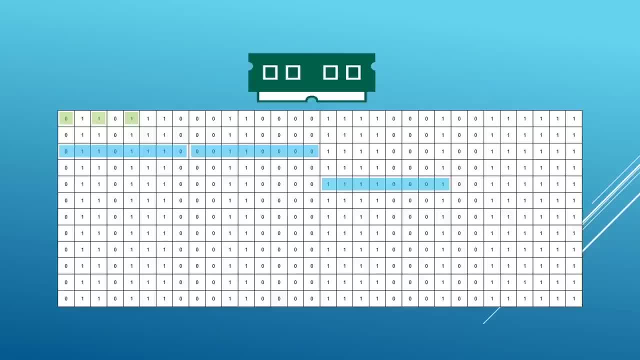 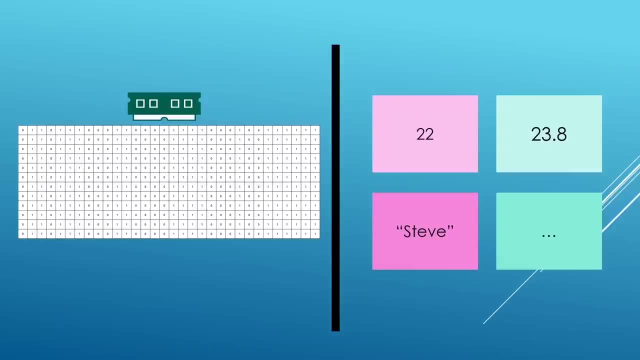 that, if you really want, you can treat each bit as a self-contained piece of data, but this is really not very useful. but there are some corner use cases for this. okay, now we really have two sides. on the right, we have data in the format that is really convenient and understandable by humans. 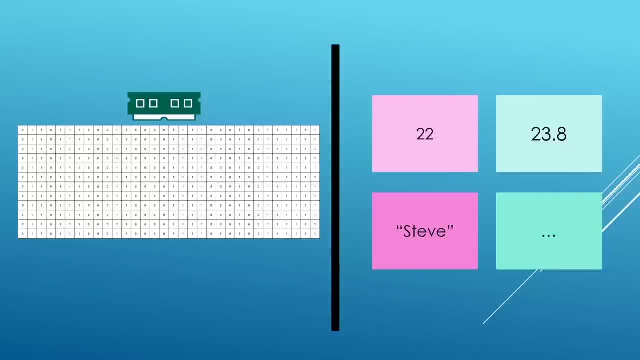 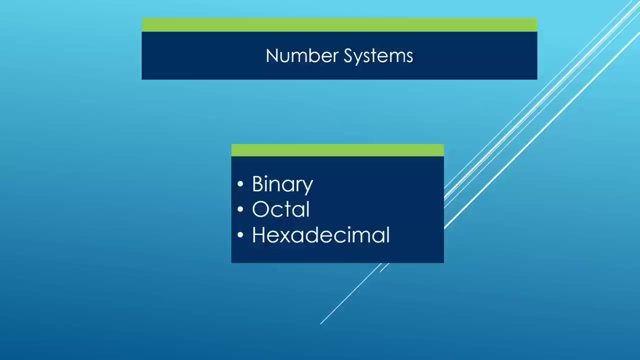 and on the left we have how data is represented in memory. so there must be a way to transform between these two forms of data, because humans can't really handle these ones and zeros well. and we do the transformation between these two representations of data using number systems. we have a few number systems available to us that we can use. 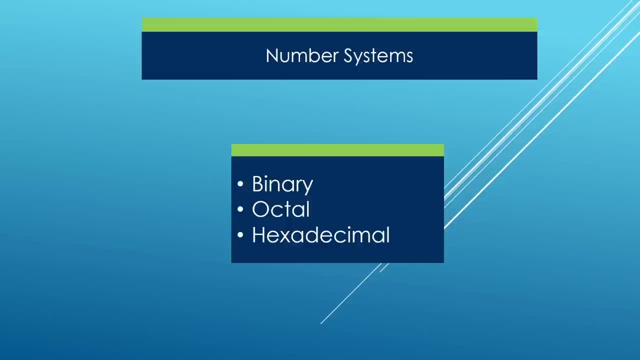 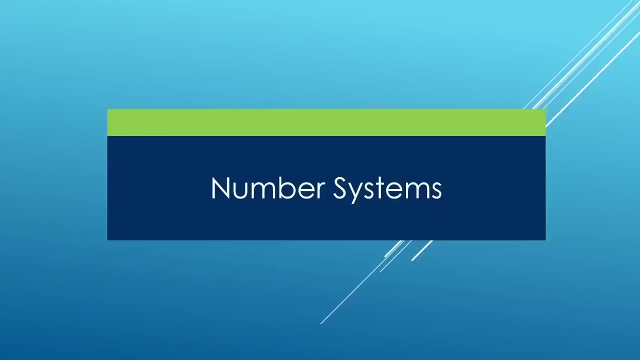 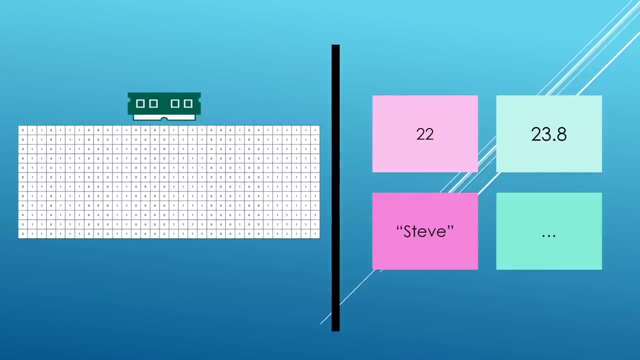 binary, octo hexadecimal are a few examples and we're going to learn about them starting in the next lecture. so go ahead and finish up here and meet me there. in this lecture, we're going to learn a little more about number systems. number systems allow us to transform data from the 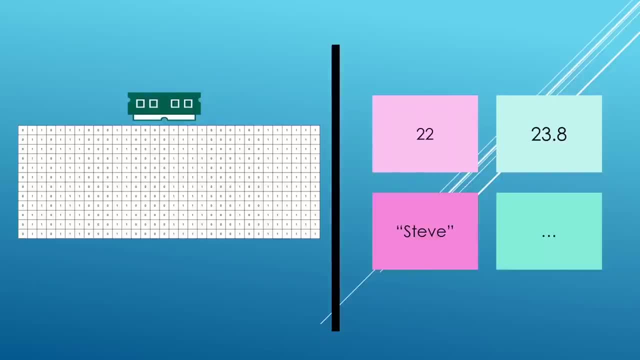 final data to the actual number systems and we're going to learn how to do this from the first lecture. form that is really convenient for humans, in a form that is convenient for computers, in these ones and zeros that you see on the left. we can also use them to do the reverse: go from ones and 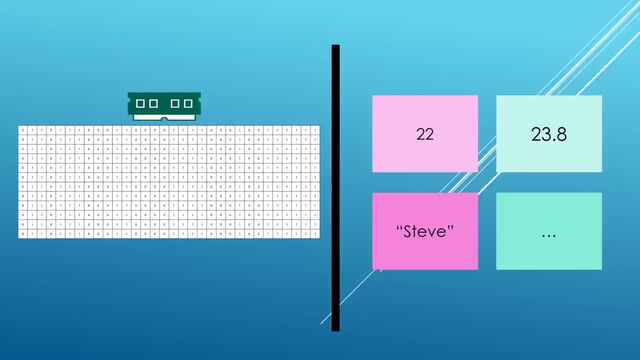 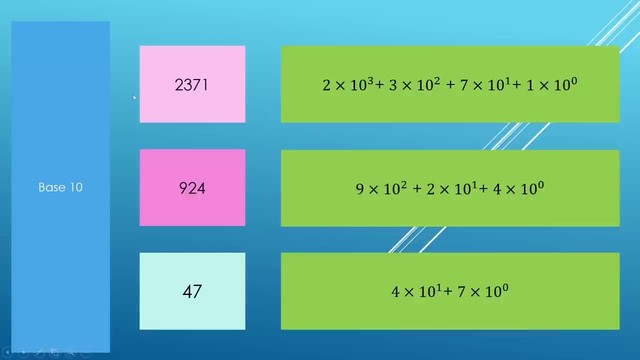 zeros and go in the format that is convenient to humans like this 22 or this steve name here, to make sense of how these number systems work, let's analyze the decimal system that we really use in daily life and that is usually called base 10.. so if you look at this 2371 number, here we can. 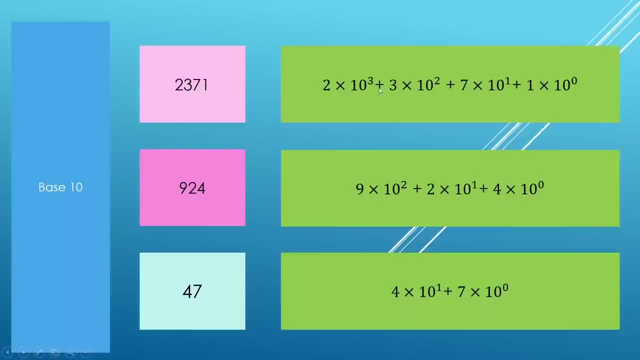 really split it in the form that you see to the right here. if you try and take this expression we have on the right here and evaluate it, you're going to get this number here 2 times 10 to the power of 3. this evaluates to 2000 and this one here is going to evaluate to 300. this one is: 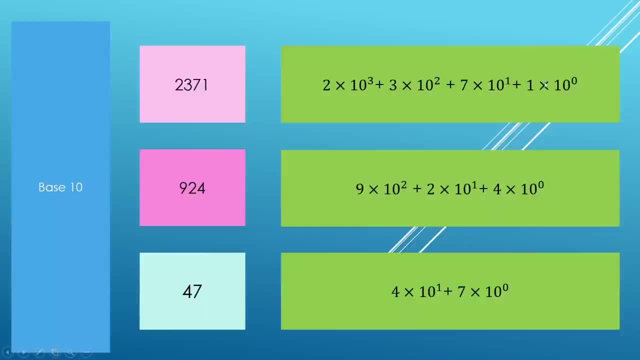 going to evaluate to 70, and the last one is going to evaluate to 70, and the last one is going to evaluate to 1, and if you add these things up, you're going to end up with this number. so this is how we can take a number and, uh, make up a base 10, representation of that. we can do the same thing. 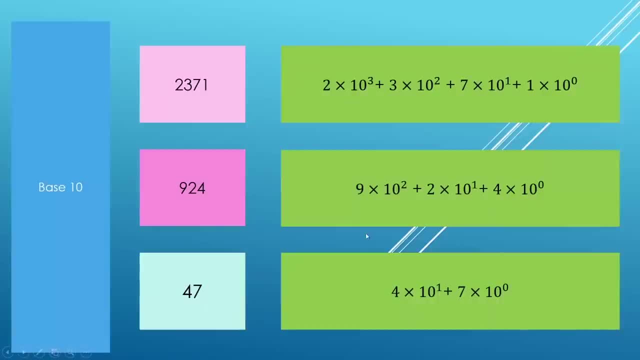 for 924 here or 47 here. it really is basic math. you don't need to have a lot of background in math to make sense of this. so we're going to use this exact form and understand binary numbers. if you look at what we have here, we have a few binary numbers that are: 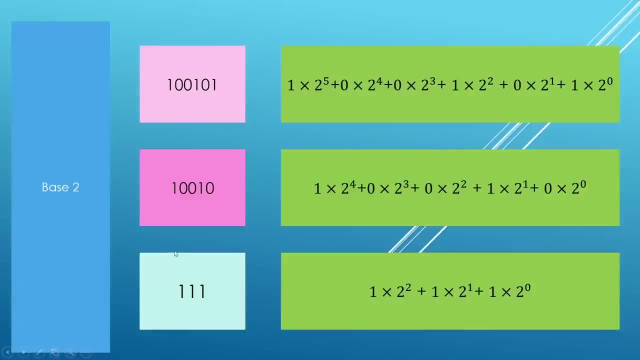 made up of ones and zeros. that's why it's called binary, because you can only have two states, or zero or one- in your numbers. so we can really do the same thing. we are in base two, so instead of using a ten here, we're going to be using it too, but it is the same operations we really did. if 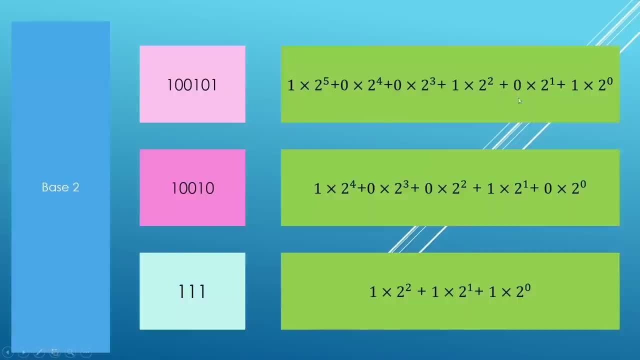 you take this and multiply and add these things up, what you're going to end up is a base 10 representation of this number. if we go in the middle here we have something we can easily do without using a calculator. the expression on the left here is going to evaluate: 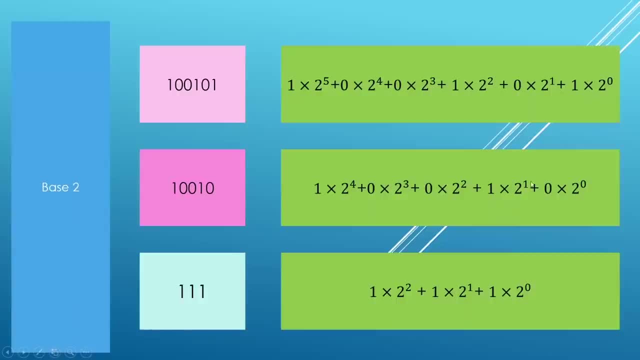 to zero, because we are multiplying with zero. the second one is going to be a two, because we are taking one and multiplying this by two. the others are going to be zeros, but the last one is going to be two to the power of four, which is sixteen, and we're going to add a two and this is going to 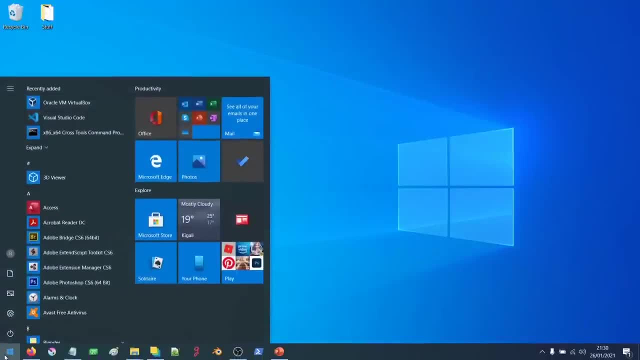 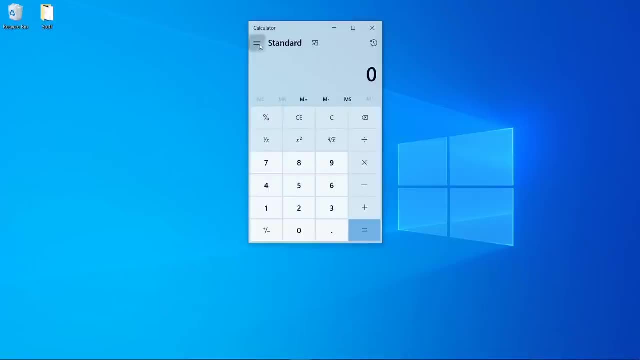 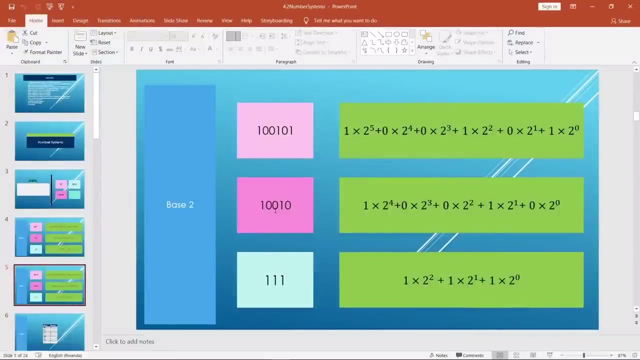 evaluate to eighteen. we can actually bring up our calculator on windows 10. i think it can help in this a little bit. we're going to bring it up and we want to put it in a programmer mode and we're going to go back on our slide and find our number, which is one zero, zero. 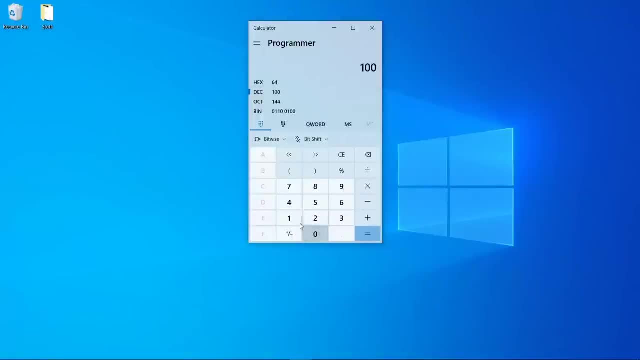 one zero. so we're going to type it out: one zero zero, one zero in binary. this is binary that we have typed here. so let's clear this and do one zero zero, one zero, and you're going to see that it's going to be one zero zero, one zero one, which is what we came up by computing this in our brain. 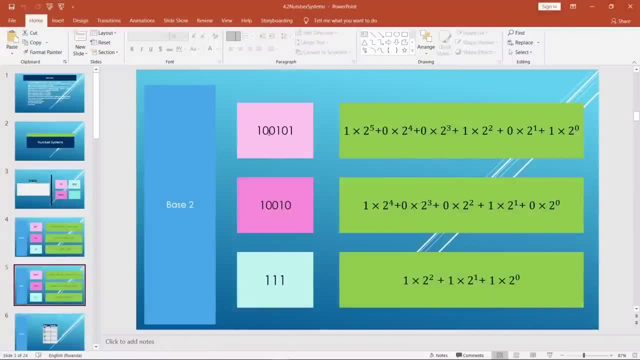 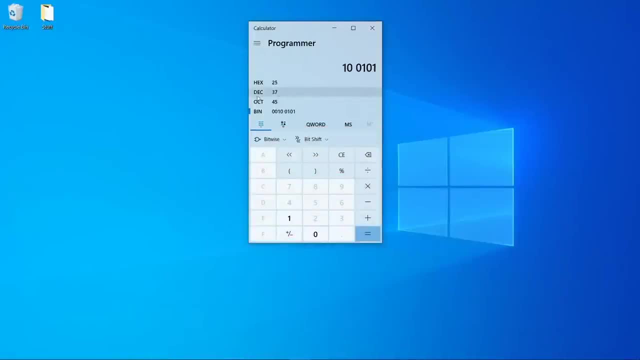 let's try the one we had before that we couldn't really do in our brain. we're going to say: one zero zero, one zero one. let's do that. we're going to clear: one zero, zero, one, zero one. this is going to evaluate to 37 in decimal and you can use calculators like this to really do the transformations. 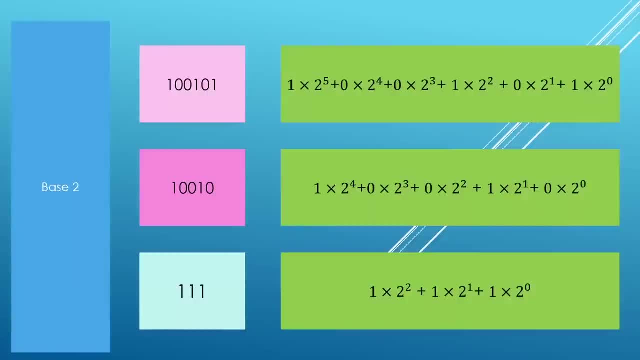 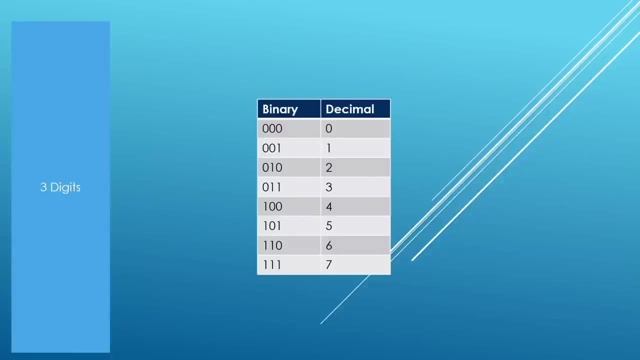 between these different number representations. okay, down below we have a one one one which is to a seven in base ten. okay, if we have three digits, we can really represent numbers between zero and seven, and you see a table here that is going to prove that zero, zero, zero is going to. 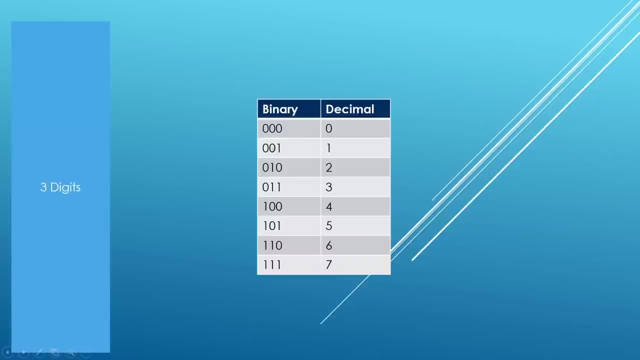 evaluate to zero in decimal. zero zero one is going to be a one. and if you go down to one one, one that is going to evaluate to a seven, you can try and use a calculator to prove this and really understand how this works. if we use the three digits representation our number. 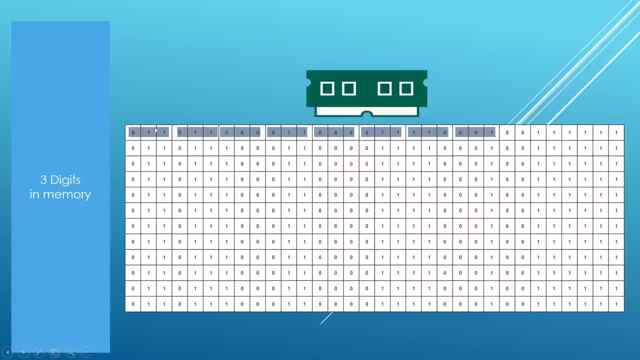 numbers are going to look something like this in memory. we're going to take the bits in memory and group them in groups of three and we are going to use binary to actually make sense of these numbers. for example, here on the left, this is going to be a one. the second one, from the left, is going to be: 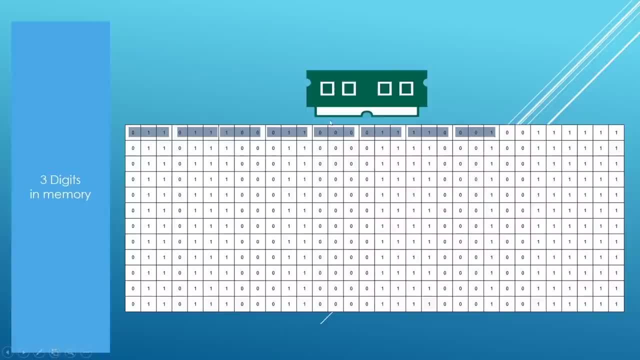 a six, and this is going to be a six as well. this is going to be a zero, this is going to be a three, because we have one and two here. we add those up, we get a three. if this doesn't make sense, you can try and use a calculator. 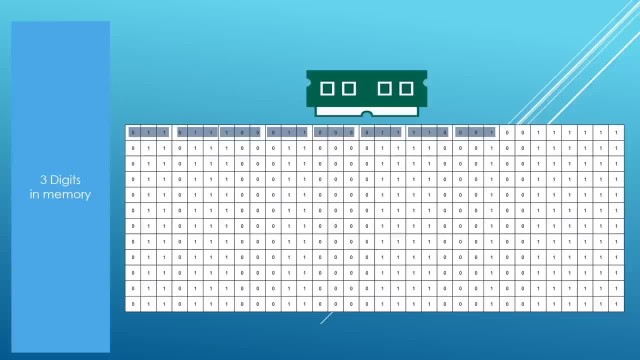 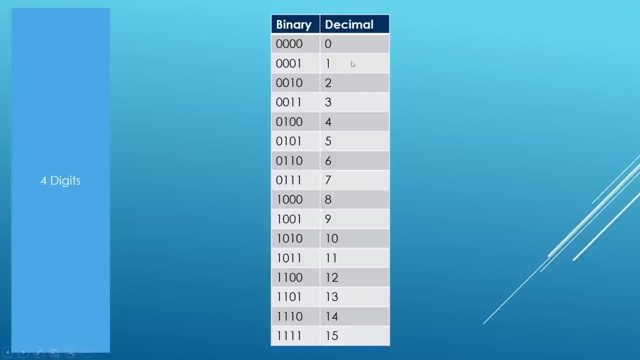 you're going to see that it makes sense, okay. so what if we want to group our digits in groups of four? we can do that, and we're going to end up with something like this: the values we can represent are going to go from 0 all the way to 15, and you can try and prove this using the calculator like: 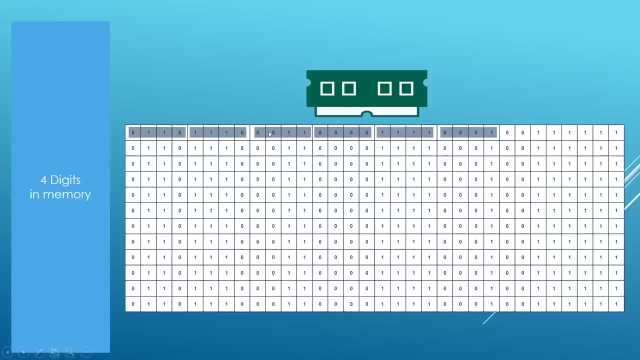 we just did and it is going to look like this in memory. so what we really are doing is grouping the bits in different sizes of data and we have a kind of formula that we can use to make sense of the data and memory. for example, on the left here we have 0, 1 1 0. if we go back to our table and define the 0 1 1 0, this is a 6, and 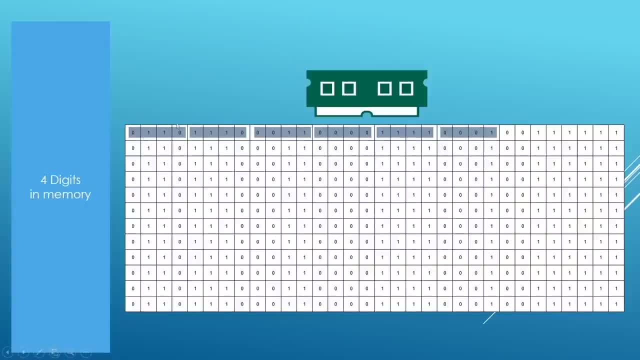 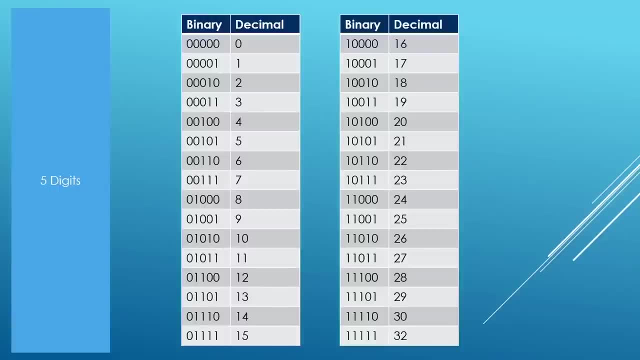 we're going to know that these four bits here are really storing a six and there are ways you can manipulate this. in your c plus plus program we're going to see that you can also use five digits and you're going to end up with something like this and the numbers are going to go from zero or 50. 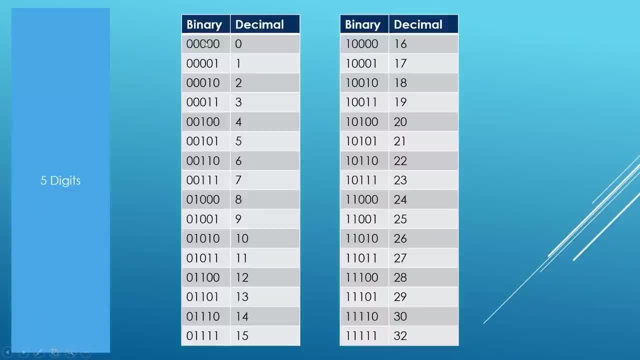 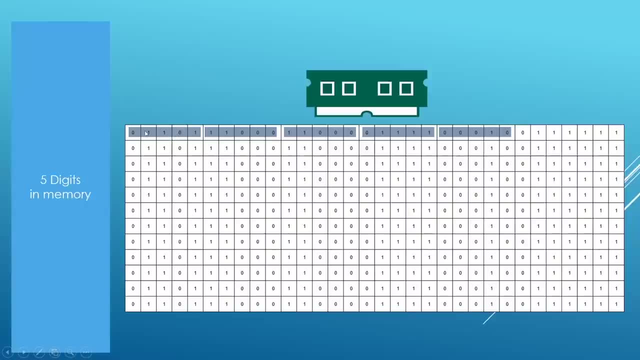 As you surprised, ours play a six. that's pretty awesome. tenis from mistake, which come end up with thatு. we're going toé all the way to 32 and this is how it's going to look. in memory you can try and come up with. 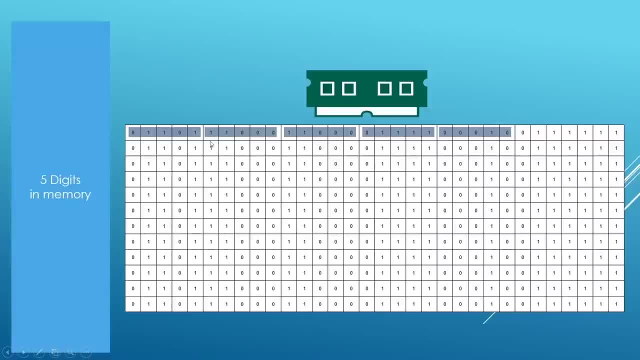 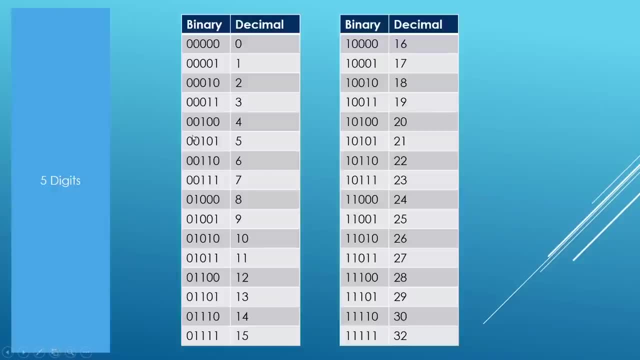 what this represents in decimal. i'm not going to tell you this, but we can try and figure out the one on the left here. so it is 0 1 1 0, 1. if we go back, we're going to come up to 0 1 1 0, 1, which. 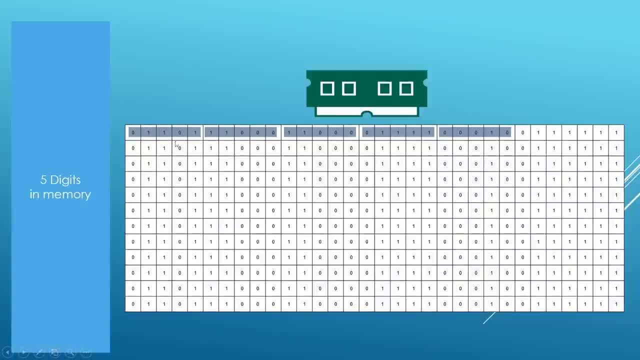 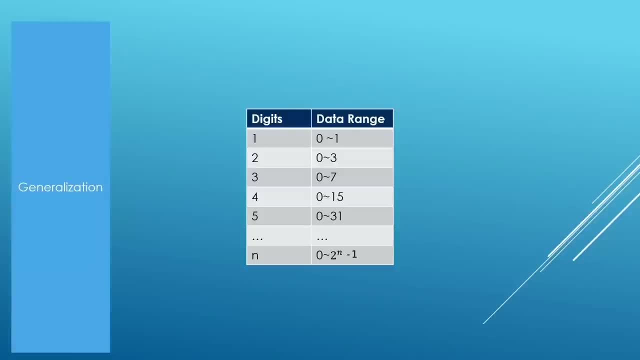 is a 13 here. so this memory location, these five bits, represent a 17 number. so if we want to kind of generalize what we have talked about in the last slides, if you have one digit you can really represent two states: zero and one. if you have three digits you can represent numbers between: 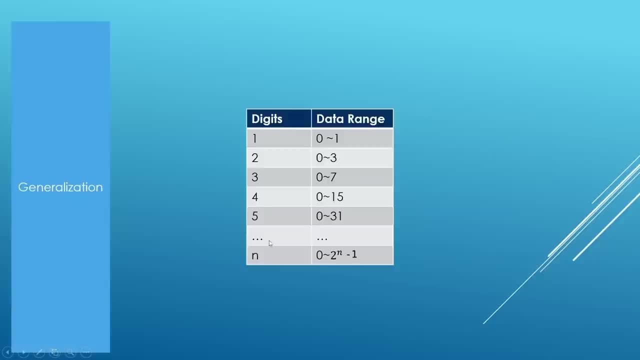 zero and seven, and you can go all the way down. and if we generalize this in a mathematical formula, we can say that if we have n digits, we're going to be able to represent between zero and two to the power of n minus one. and if you try to plug in any number of 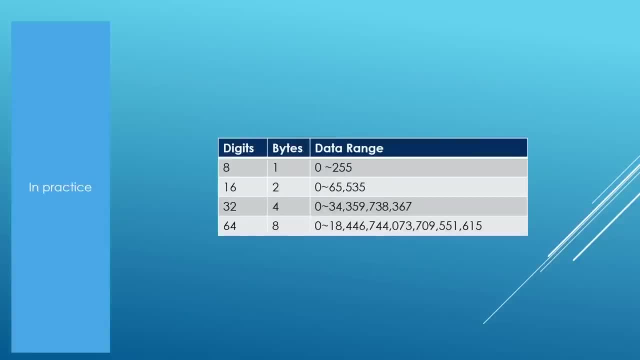 digits. you're going to see that this formula works okay. so these are a few grouping of bits we have in practice. we can use eight digits and we can represent numbers between zero and two, five, five. if we have 16 bits, we can represent this range. if we have 32 bits, we can represent this. 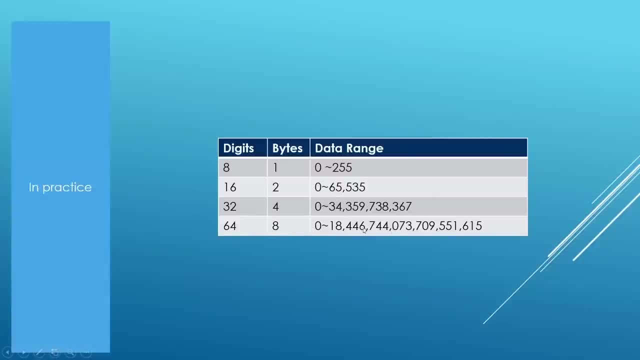 range. if we have 64 bets, we can really represent a really huge range. i can't even say this number, it's really bad. okay, now you should have a pretty good idea of the binary system and different representations we can use to make sense of binary numbers in a computer's memory. the last thing i want you to see is what we call hexadecimal. 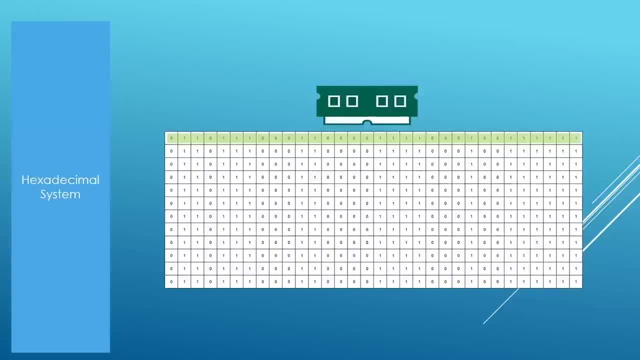 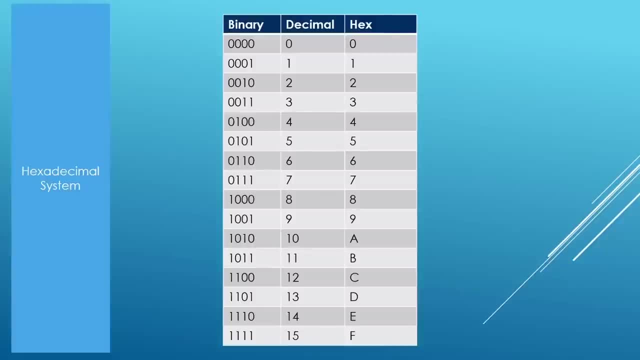 number system, and it is a technique we use to shorten the length of how we represent a binary number in memory. how does it work? well, we take our number and split it in groups of four bits, and each of the numbers is a number of four bits, and each of the numbers is a number of four bits. 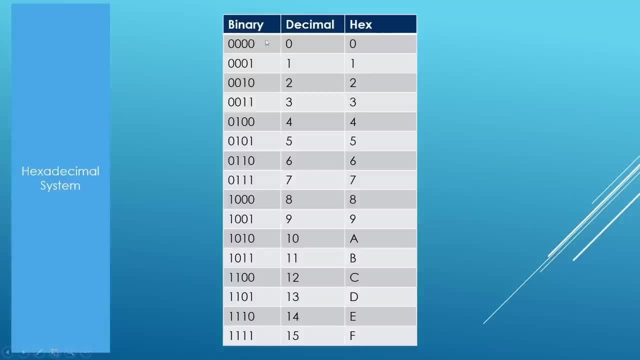 each group is assigned a symbol we can use to represent it. if we have four zeros, that's going to mean a zero in hexadecimal. if we have zero, zero, zero, one, we're going to represent a one, and you can see that if we go up to nine, this is really similar to what we have in the decimal number. 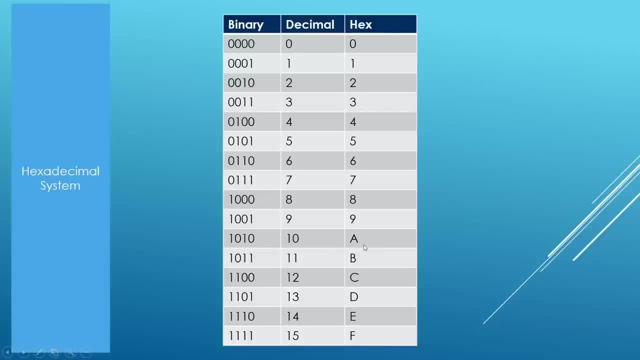 system. but once we hit ten, we're going to represent that with an a in hexadecimal. eleven is going to be b, twelve is going to be c, thirteen is going to be d, fourteen is going to be e and 15 is going to be f. so how do we use this to represent binary numbers? let's see an example. 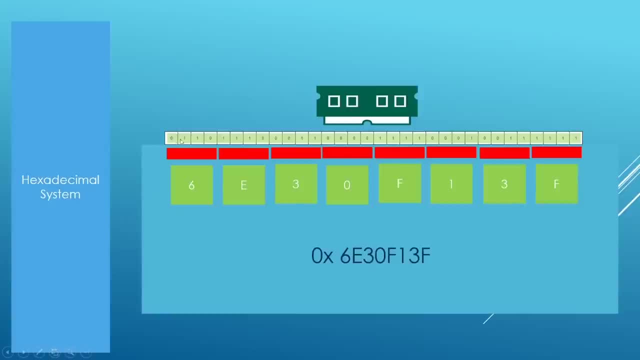 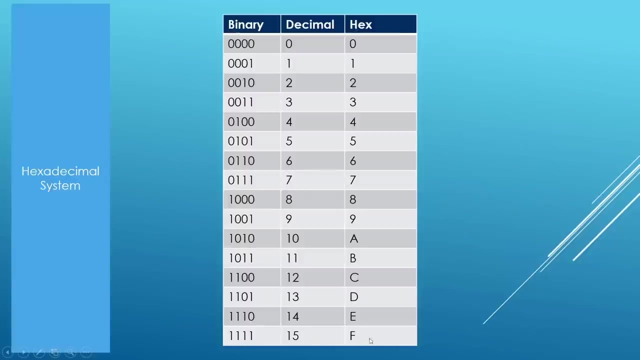 here we have a huge number that we represent in memory. it starts with zero and ends with the one here. so the first thing we're going to do is to split this in groups of four, and the one on the left is going to be a one one, one one. if we come back to our table here, one, one, one, one means f, so 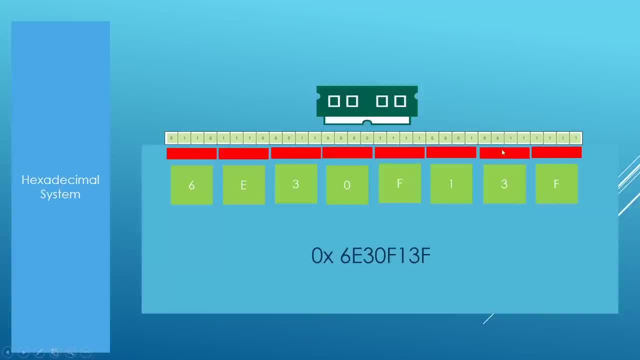 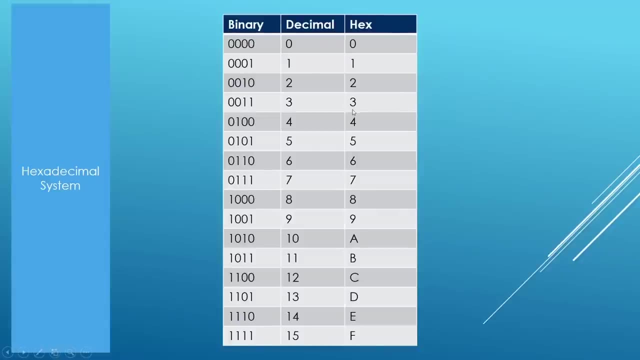 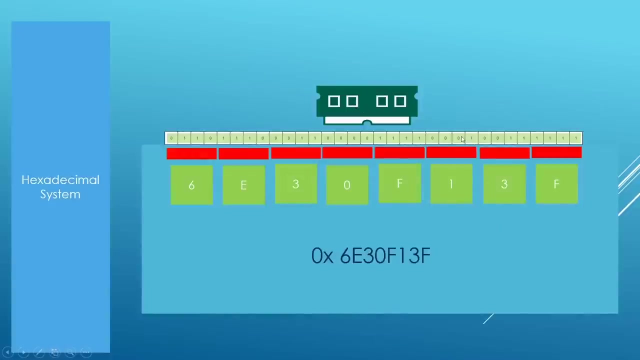 we're going to represent this with an f. if you go to the second group of four bits, we have zero zero one one. if we go back, zero zero one one means three, so we're going to have a three here. i hope this makes sense and we're going to keep using the same transformations and we're going to come up. 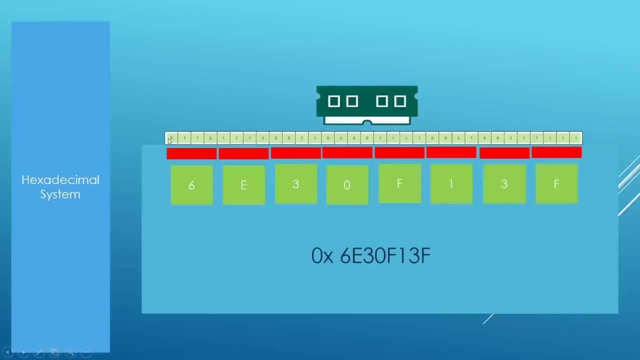 with one f, zero, three, e, six, and we can represent this binary number using these symbols. you can see that we go from using 32 bits to using one, two, three, four, five, six, seven, eight symbols to represent this, and this is shorter and easily manipulable by humans. and we use a zero x in front to mean that this is a hexadecimal number. i really 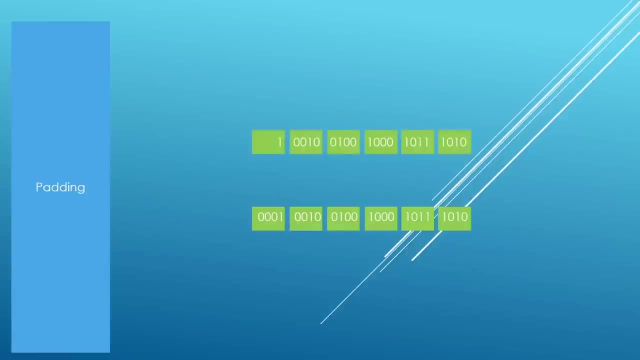 hope this makes sense. so if we have numbers that don't really fit in groups of four, we're going to go from the left and split this in groups of four and we're going to end up with a group on the left that doesn't really meet our requirements. 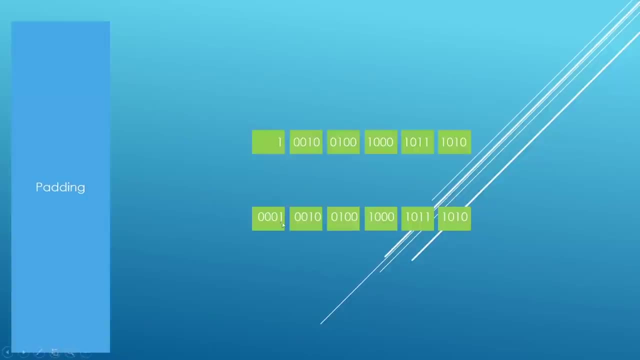 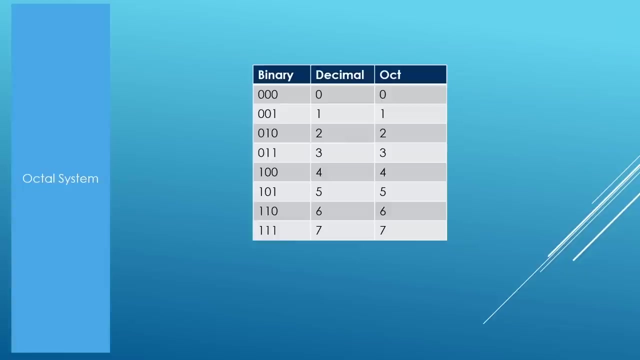 and what we can do is add the missing bits and make them zeros, and we call this operation padding. this is what you can do to really represent any number in hexadecimal if you don't have enough bits on the left. we also have another system that is really not widely used today, but i am mentioning 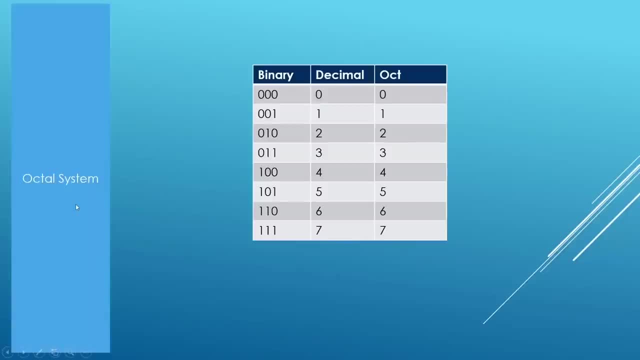 it here for completeness, it is called octo system. it goes from 0 all the way to 7 and we can divide our binary number into groups of four, of three and represent using these zeros and ones to shorten the length of the binary number we can. 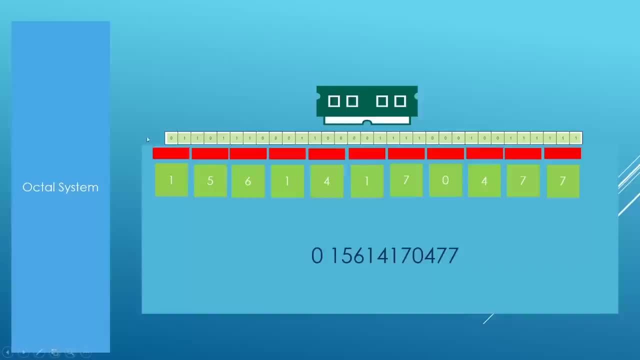 really do the same thing we did with hexadecimal, so we're going to take our binary number and divide this in groups of three. the one on the left is going to evaluate to a seven because it's one, one, one and one one one evaluates to seven in octo system. the second one is also going to be a one. 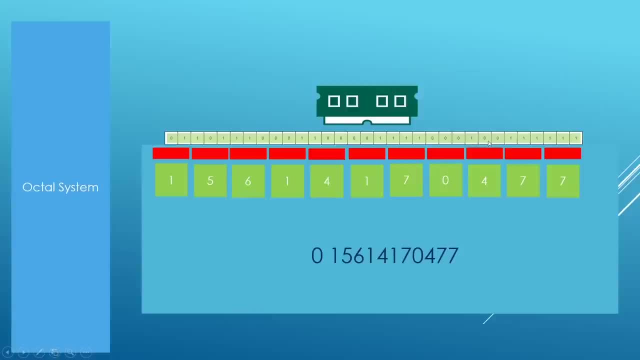 one one. the third one is going to be one zero, zero. if we go in our table it's going to be one zero zero. it's going to be a four and you see we have a four here and you can do the same things until you have figured out the entire number here and you see, on the left we are doing. 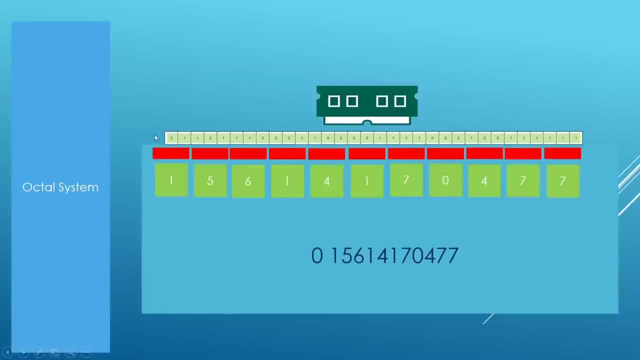 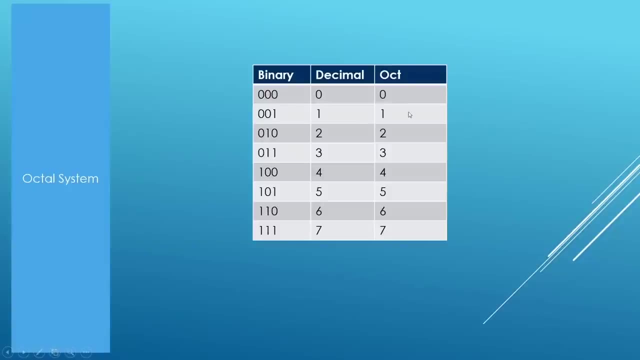 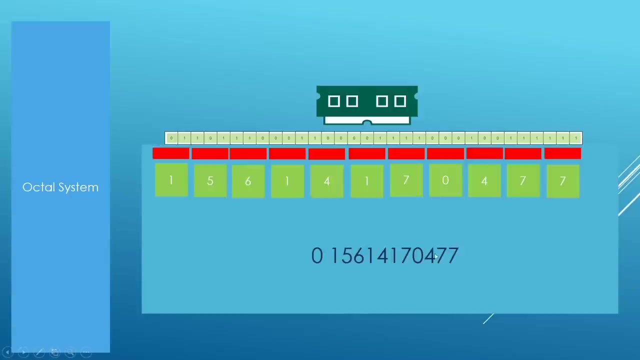 padding and adding a missing bit and making it a zero. so we are coming up with zero, zero one and if we go back to our table here, zero, zero one is a one and that's what we put here. so we're going to put this number here. it's going to be fifteen, sixty one, forty one, seventy forty seven, seven. 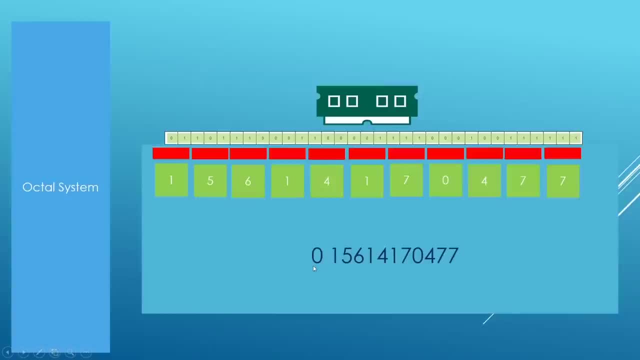 zero in front, to mean that this is a number represented in the octo system. i really hope this makes sense. okay, so we have seen all these binary numbers and different number systems we can use to represent them, but how do we use them in a c plus plus program? well, i'm glad you asked. 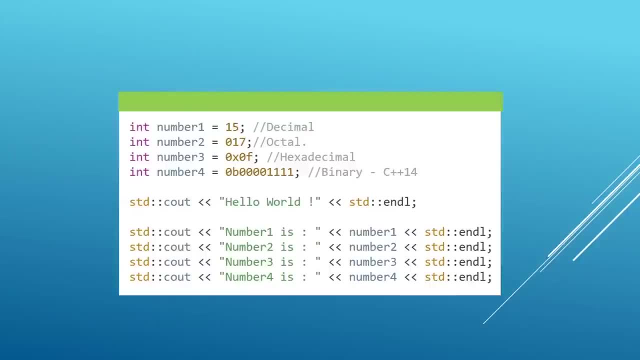 here is a simple example of how you can represent the number 15 through different number systems. in c plus plus, if you just say 15 like this, it's going to be in decimal. if you add a zero in front, it's going to mean that the number is in octo system. so this can be. 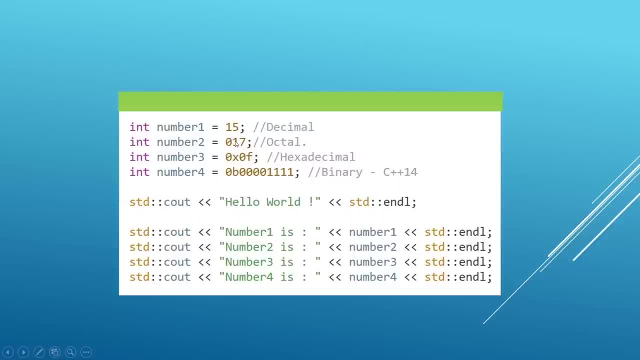 confusing sometimes. if you do 017, it's not going to be 17.. so if you say 017, c plus plus is going to interpret this number as if it is in octo system and it is going to turn this into 15.. down here you see the same representation in hexadecimal. we saw that you use a zero x in. 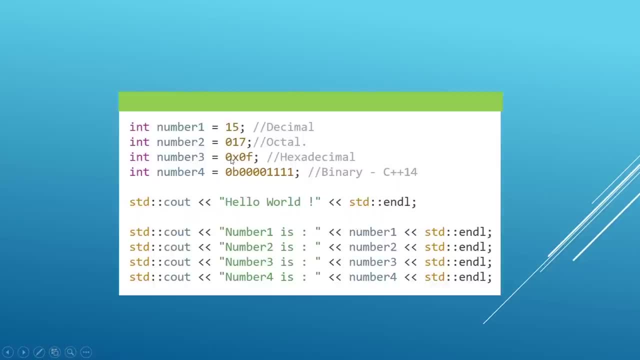 front to represent that it is in hexadecimal. and uh, this is the same representation in hexadecimal, going to be 15 in memory. and here we have a representation in binary using zeros and ones, and you use 0b in front like this. i have to say that this was only possible since c plus plus 14. 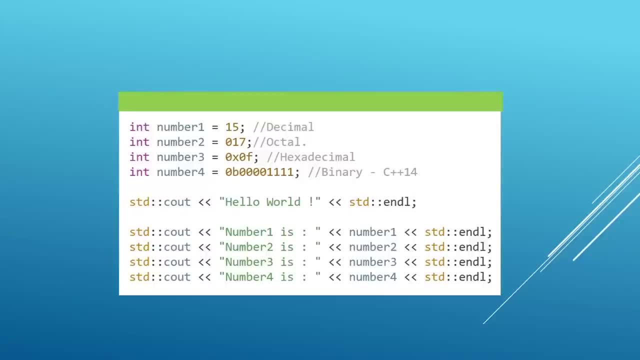 so if you are using an older standard of c plus plus, you won't be able to represent binary like this. and if we run this program, it is going to print the same thing. it is going to print 15, but we stored the number using different number systems. let's go to visual studio code. 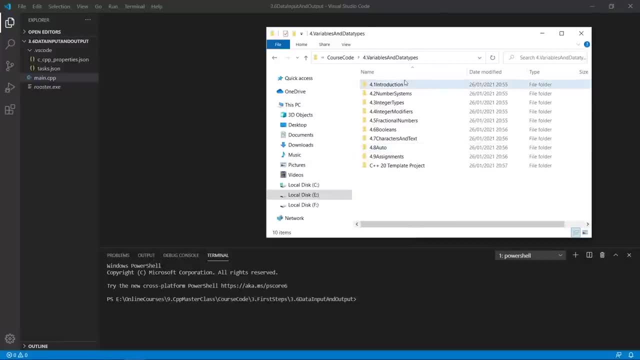 and we're going to use the same thing. we're going to use the same thing. we're going to use the same. try this out. okay, here we are in a folder i have on my system where i am going to be storing my projects for this chapter. the first thing i am going to do is copy code from a template project. 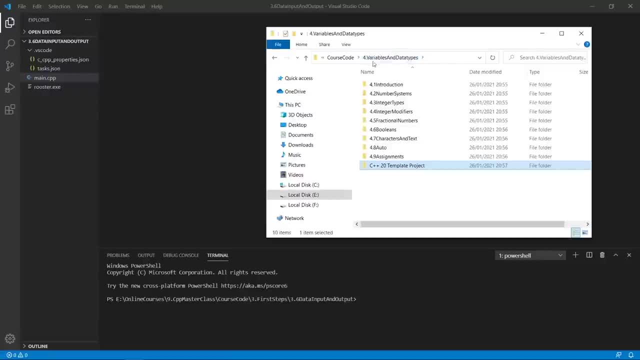 i am going to go in and copy things over and i am going to put these in for two number systems. i am going to open this folder in visual studio code, so i am going to go to file, close the folder we have now and i am going to open up a new one. open folder and then. 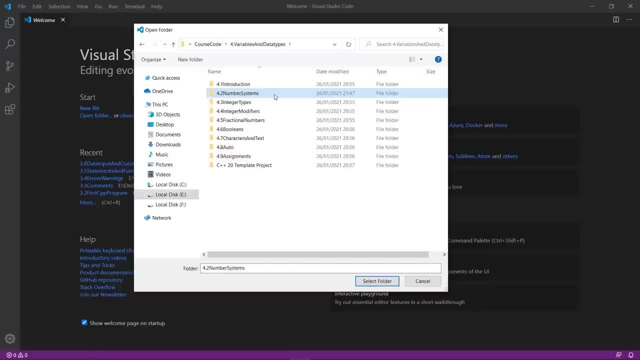 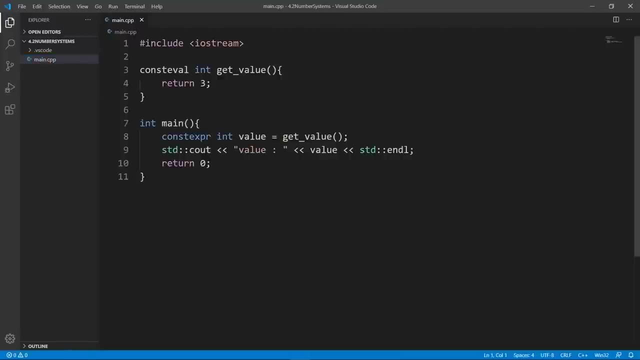 i'm going to browse to the location of my project. i am going to open this project here that says number systems. we are going to get rid of the welcome screen and open our main cpp file. we're going to get rid of this const eval thing and clear everything we have in the main function. 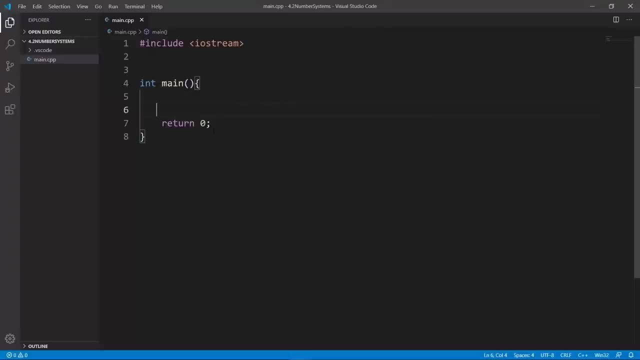 here, the first thing we want to do is to store an integer that is 15, and we're going to say int number one- the exact same thing we had in the slides- and we're going to store 15 in this variable. here this is going to be represented in decimal, and if we want to store the same number, 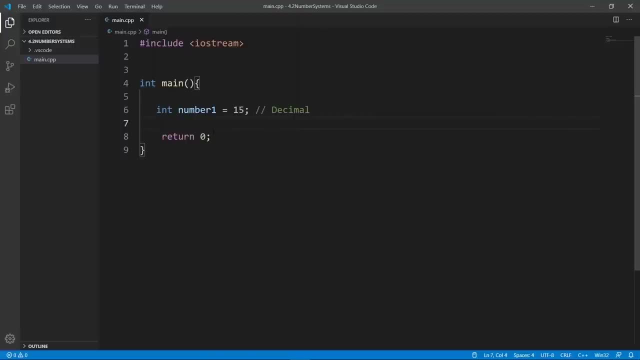 in octal. we saw that in our slides we could store this as 017. so let's do that. we're going to say in number two and we're going to store in 017. this is not going to be 17, this is going to be a. 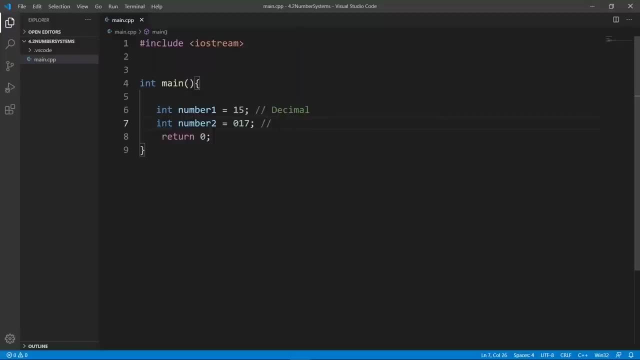 representation of number in octal system. so we're going to say that this is octal and we can store in hexadecimal as well. so we're going to say int number three, and it is going to be 0x because it is hexadecimal, and we're going to say 0f. this is how we represent it. you can use lowercase. 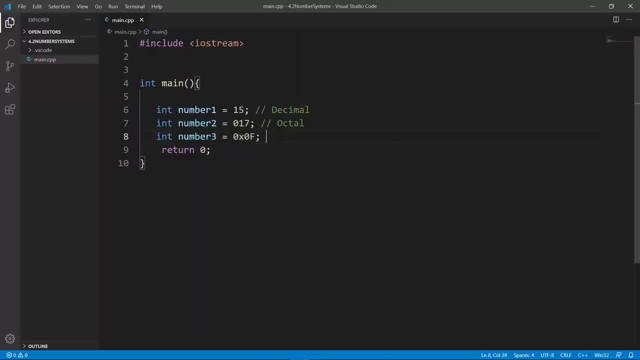 or uppercase, it won't really matter. let's use uppercase here and we can use binary because we are using z plus plus 20.. so we're going to say int number 4 and we're going to store in a representation of 15 in binary, and it happens to be four zeros and four ones. 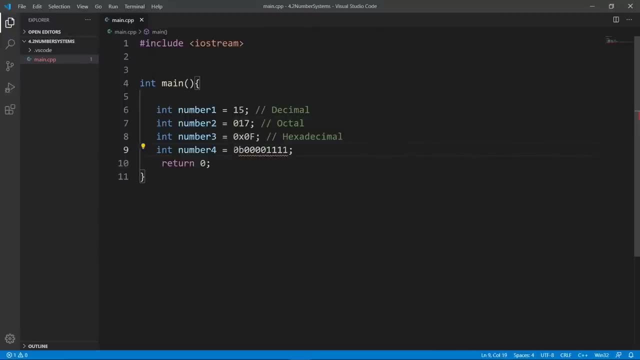 and we have to prefix this with a zero b. this is how it works. so this is going to be in binary and if we print all these numbers up, we're going to see- let me not tell you this- what do you think we'll see. okay, so i went ahead and typed this out: what do you think we will see when we build and 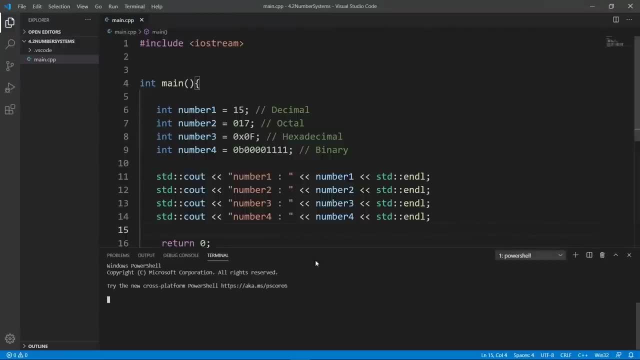 run this program. before we do that, we're going to open a terminal so that we see it here and we're going to go to terminal run task. we're going to build with gcc. let's go to gcc. let's wait and see if the world is successful. world finished successfully. we have our rooster. 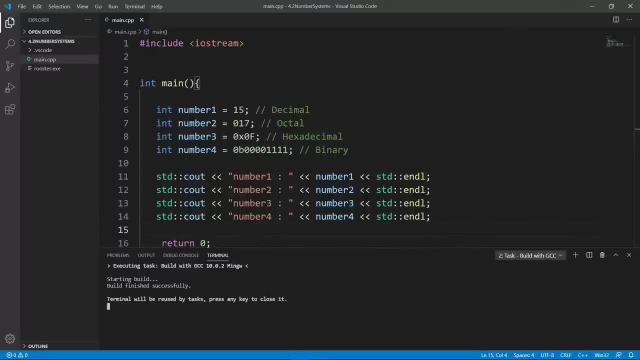 program in here. we're going to click somewhere in this terminal and our terminal is going to show up. if we do there, you're going to see that our rooster program is here, and if we run it, i want you to take a moment and guess what we're going to see? hmm, number 1: 15 and number 2: 15, and 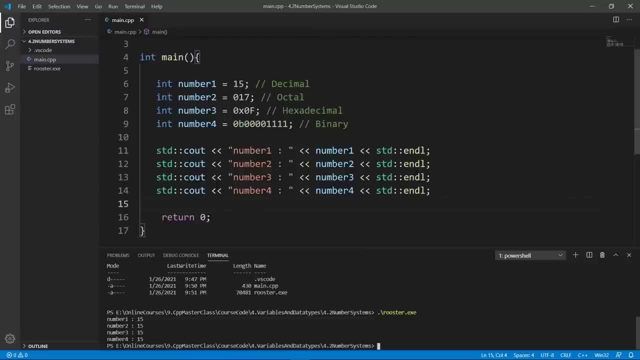 number 3: 15 and number 4, 15.. this is really the same number we are storing in this variables, but it's going to be a different representation that is going to be convenient, depending on whatever it is we are doing. if it is more convenient to use binary, we're going to use binary. if it is more. 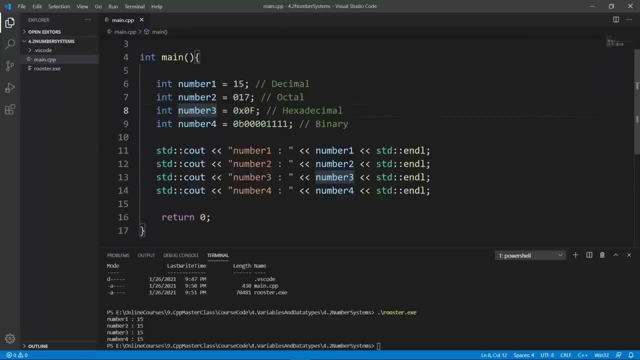 convenient to use hexadecimal, please do use hexadecimal, but the representation of this number in memory is really going to be the same. i really want you to take some time and let this sync in, because you're going to see these things a lot of times in your career as a software developer. 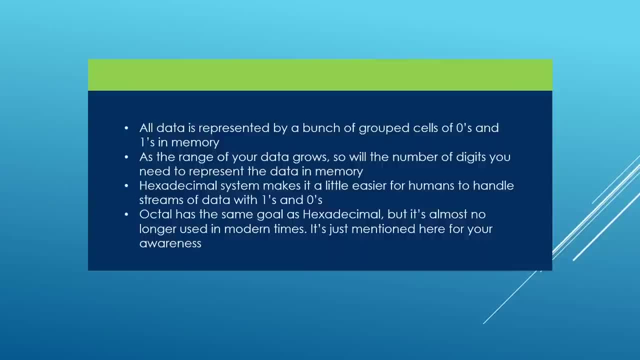 and make sure you really understand this. okay, this is really all we set out to do in this lecture: trying to make sense of the binary numbers we have in memory and how we transform between them and different forms of data that is easily manipulable by humans. all data is represented. 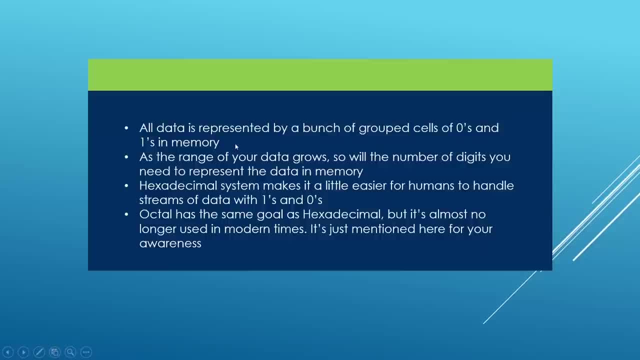 by a bunch of grouped cells of zeros and ones. we have seen this. as the range of your data grows, so will be the number of digits you need to represent the data in memory. we have seen that the hexadecimal system makes it a little easier for humans to handle streams of data in ones and zeros. octo has the same goal as 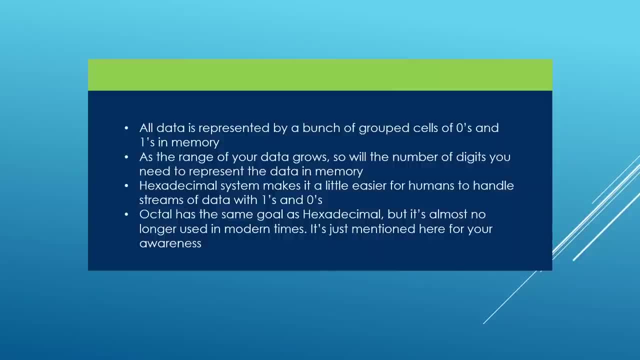 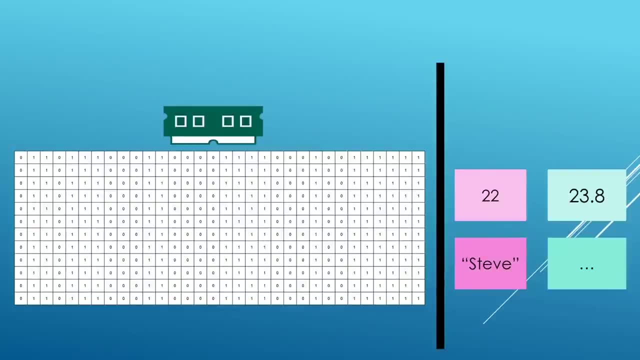 hexadecimal, but it's almost no longer used in modern times. i just mentioned it here for completeness. we are going to stop here in this lecture. in the next one we're going to look at integers in a little more detail. so go ahead and finish up here and meet me there in this. 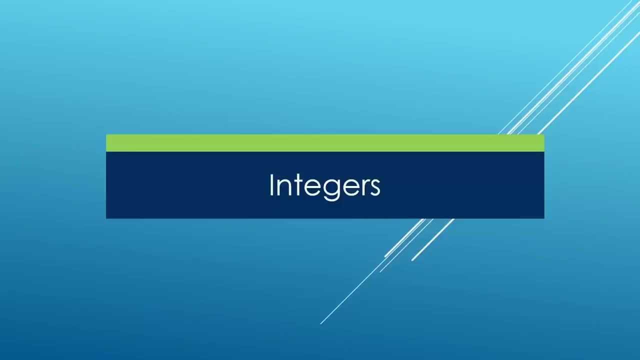 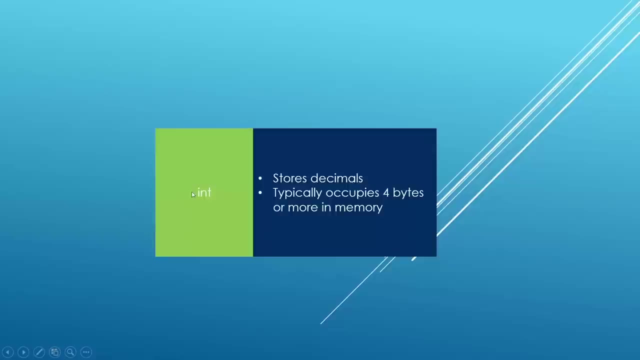 lecture we're going to learn a little more about integers in c plus plus. integers are represented by ent in c plus plus- it's what you see on the left here- and they are used to store whole numbers, things like one, two and three. they typically occupy four bytes or more in memory, but in most 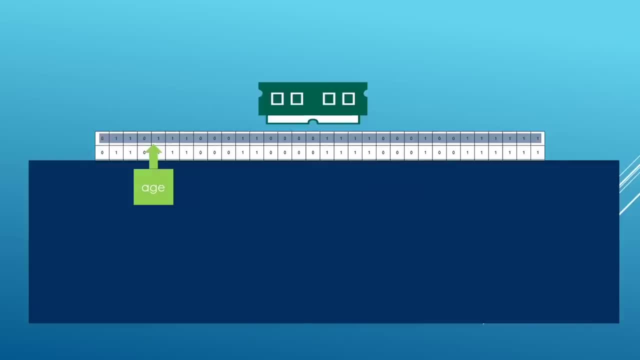 times it's going to be four bytes. so, for example, if you have a variable called age and it is an integer, this is how it's most probably going to look in memory. it's going to take four bytes and i really want to make it clear what the variable is. it is a named piece of memory that you 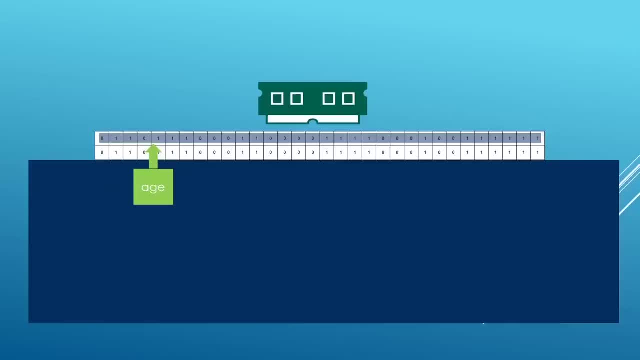 use to store specific types of data. okay, so here, if we have a variable named age, it is a named piece of memory, age is going to be the name of that piece of memory and we can store data in that memory. it's going to look like this in memory, but the value is going to be stored in here in. 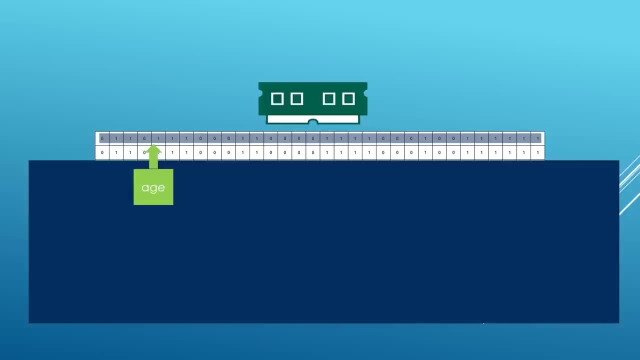 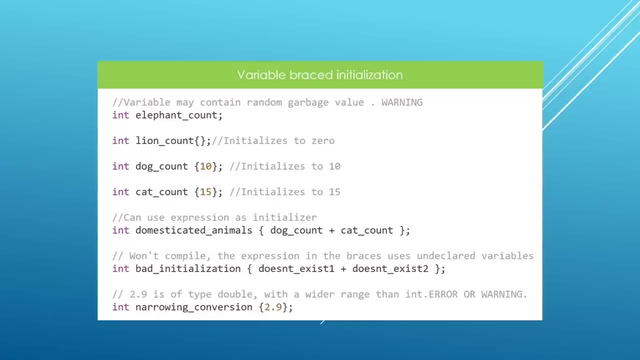 binary format. i really hope this makes sense. a variable is the named piece of memory that we can use to store different kinds of data. and okay, now we're going to look at a few examples of how you can work with integers. in your c plus plus program, you can define a few variables here. 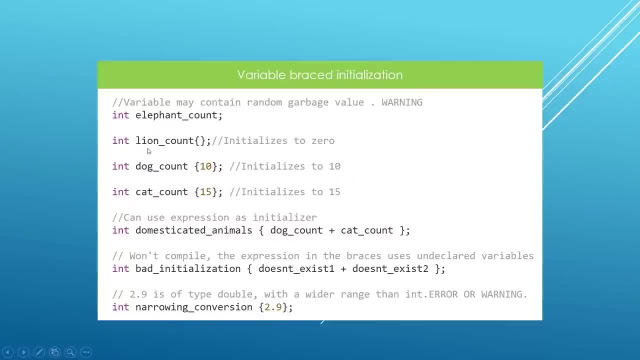 we have one that is going to store the number of elephants we have. you can declare it like this and not put in a value, and if you do it like this, the compiler is just going to put in some garbage value. that is really not meaningful for your program. so you see the warning we have here as a comment. 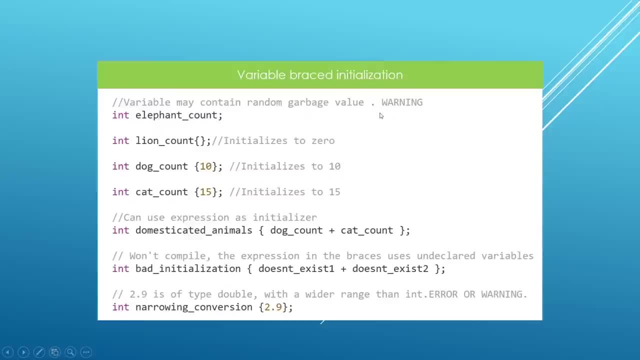 the variable may contain random garbage value, and this is something you need to be aware of. another way we can define integers in our c plus plus program is this statement here that declares a variable called lion count. it's going to initialize to zero. if we use curly braces like this, it's going to initialize to zero by default. we can also: 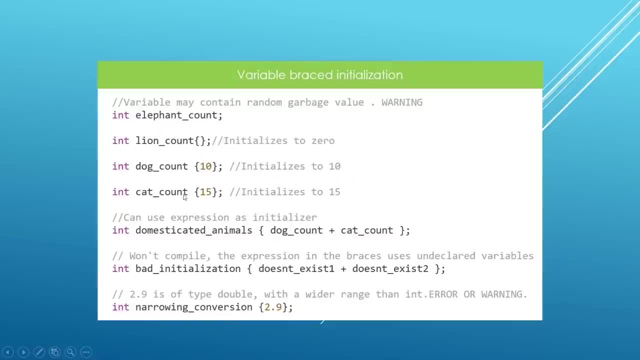 explicitly put in a value. we can do the same with cat count and we can use these variables to do operations. for example, we can declare another variable and it is going to store the number of domesticated animals and we're going to add up the numbers for dogs and cats and we're going to 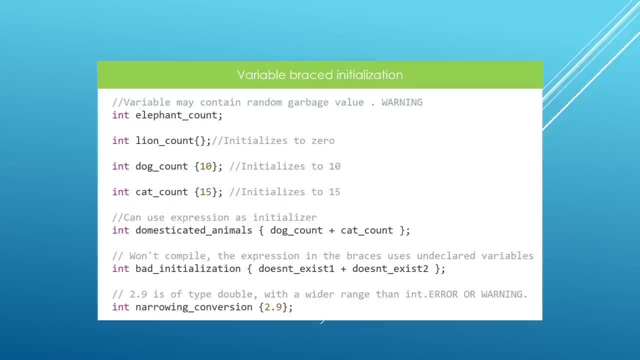 store the result of that in our variable that is called domesticated animals. this is something you can do. another thing that can be problematic is trying to use variables that you haven't defined or declared in your program. that is going to give you a compiler error, and the compiler is basically: 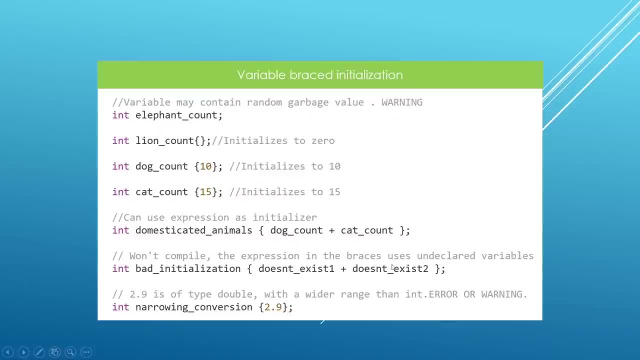 going to say: i don't know what doesn't exist. one here is: i don't know what this doesn't exist to is. it is not defined anywhere in the program. another thing you can do is try and store a fractional number in a variable that you declared as an integer, and this is going to give you a warning. 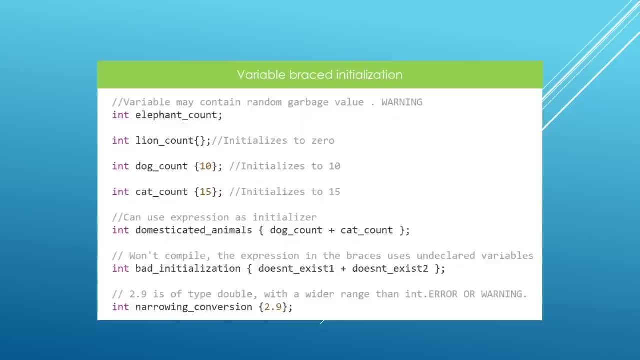 because fractional numbers are usually bigger in size than integers and this is going to lose some of your data. we don't really have enough tools to understand this now, but we are going to understand this a little later in the course. but this is something you can do. you can take a fractional 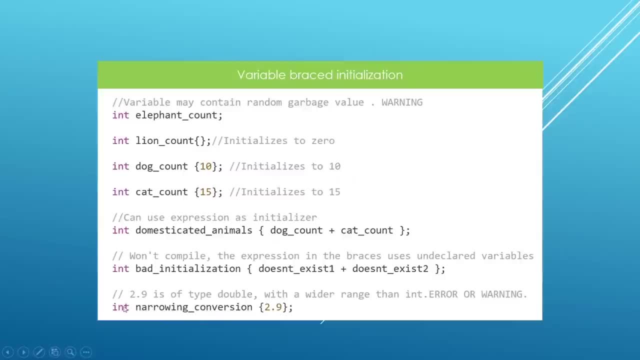 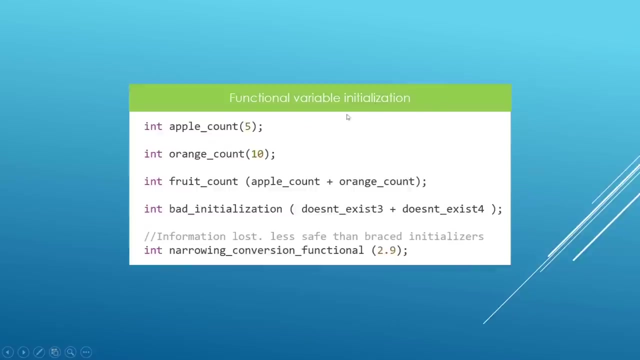 number and store that in an integer variable, and we're going to do an example and see how this behaves with our compiler that is gcc10. okay, here we have mostly used curly braces to initialize our variables, but we can also use parentheses, and this is going to be usually referred to. 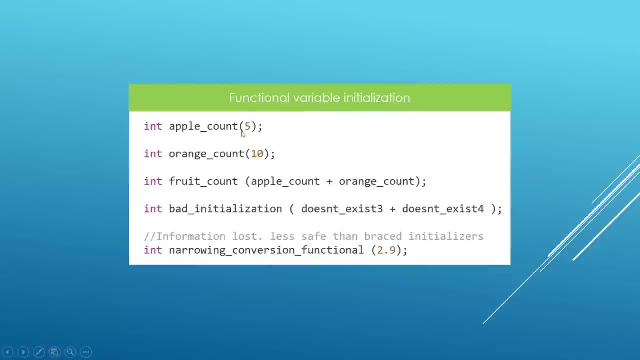 as functional variable initialization, because we are using parentheses and this is mostly going to do the same thing we saw in the last slide with curly braces. but when we come to the example here where we are storing a fractional number, this is going to silently chop off the data you have in a fractional number and turn that. 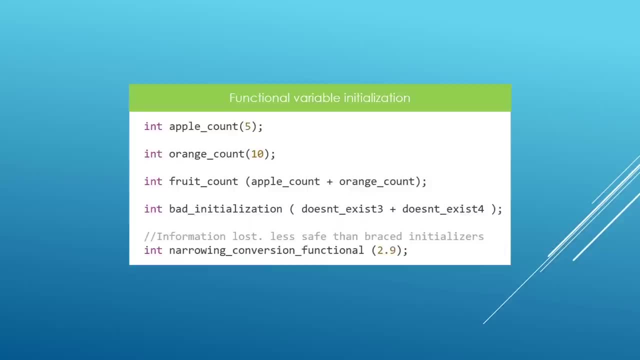 into an integer, and this is called implicit conversions. but if we go to the last example here, where we are storing 2.9 into an integer, this is going to take this fractional number, chop off the decimal point and only store 2 in this integer, and this might not be what you're. 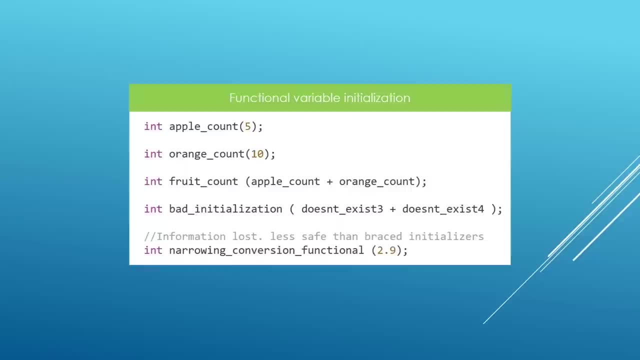 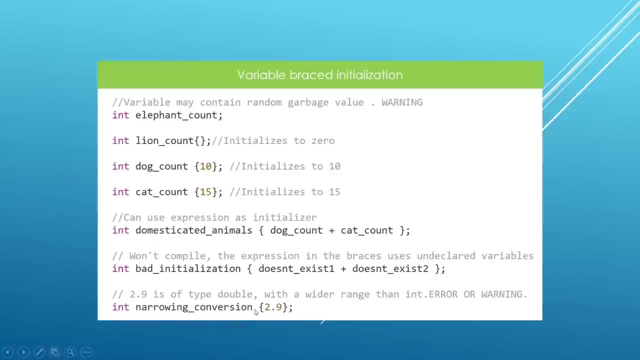 want, and it is going to happen silently, so this is a really bad way to do this. if you want to do something like this, it is preferable to use curly braces, because you are either going to get a warning that this is going to lose you data or you're going to get a compiler error and the 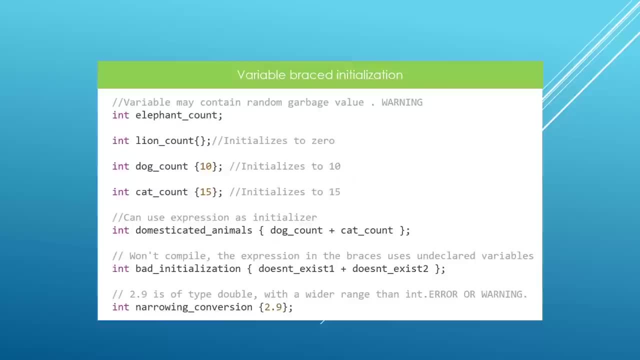 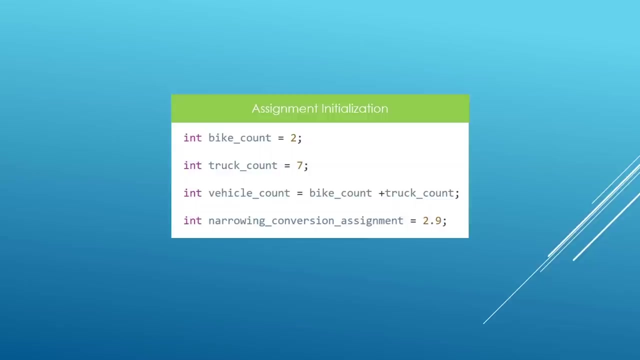 compiler is going to completely stop you from doing this. and again, if any of this doesn't make any sense, we're going to go in visual studio code, play with us and see how the compiler behaves with these things. we have another way. we can initialize our variables in c plus. plus we can use assignment. 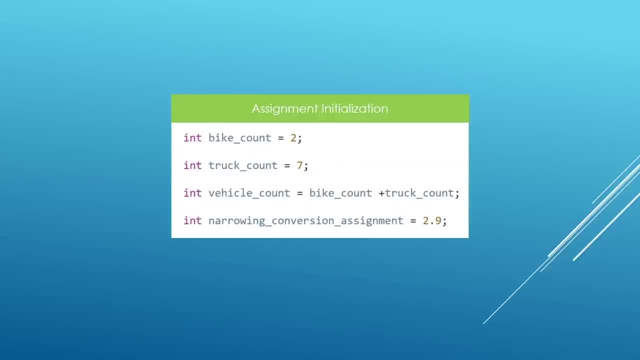 and we have done this a couple of times in the course, but this is something you can do and we are going to play with us in visual studio code in a minute and you're going to see how it works. okay, by now we have seen three ways we can initialize our integer variables. we can use 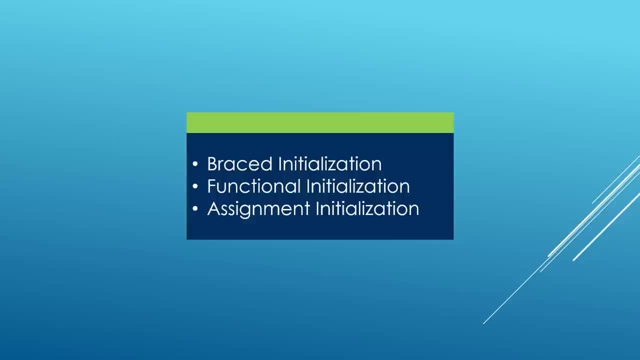 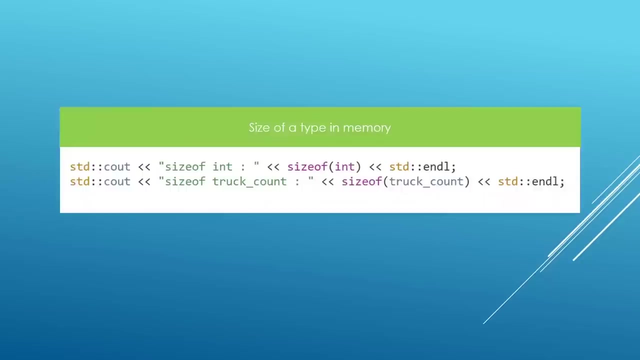 braced initialization, which is basically using curly braces. we can use functional notation, which is using the parenthesis, and we can use the assignment initialization, which is what we have here. another thing i really want you to see is that it is possible to query for the size of your variable. here we are trying to print the size and integer. 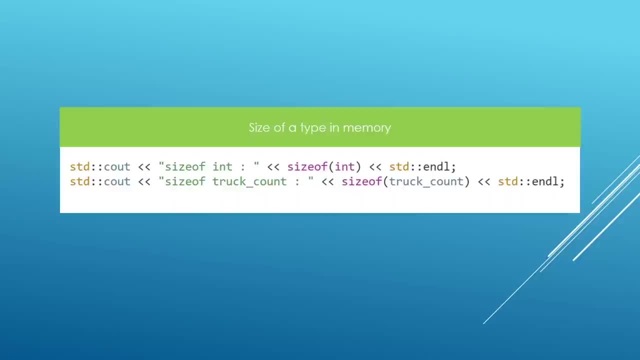 is going to take on our operating system and compiler and if you try to run this on our compiler, it's going to tell us exactly how much memory an integer occupies. in our program we can either pass int explicitly, like this, or we can pass a variable name, and it is going to work. 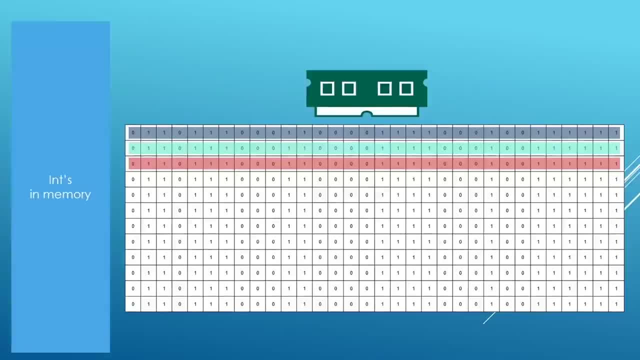 equally well, okay, ants are mostly going to take up four bytes in your memory. so here we have a representation of three ants in memory. if we go from this zero to this zero, this is going to be exactly four bytes, and uh, this is how it may look in memory. one other thing i haven't really. 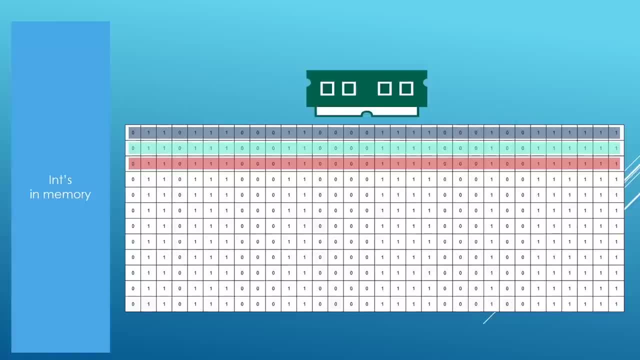 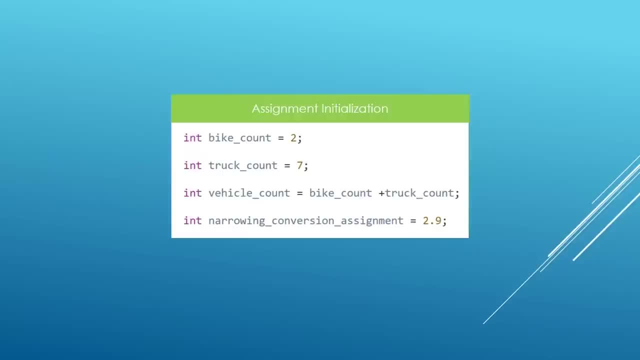 talked about on purpose is that there are a few rules you have to follow to name your variables in plus plus. one of those rules is that a variable must start with the letter like a, b, c, d up to z or an underscore. you can't start a variable, for example, with a number. that's going to be a problem. 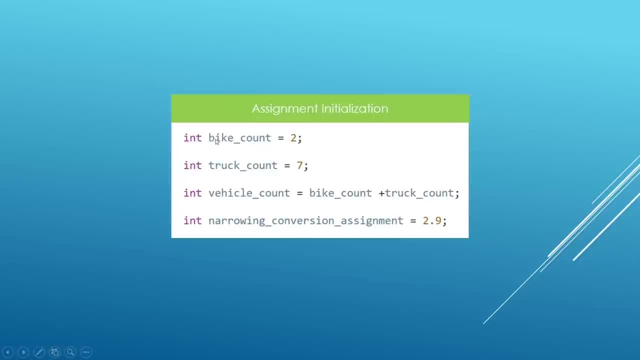 after the first character in your variable name. you can really put in anything. you can put in numbers, you can put in letters, you can really put anything you want, but the first one can't be a number. variable names are also case sensitive. so if you have a variable called 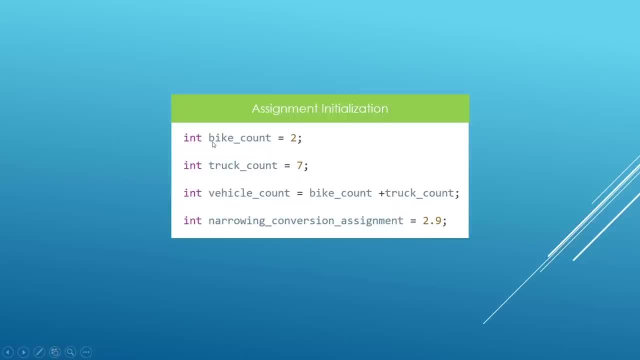 bike account with the lowercase b and you have another one that starts with uppercase b. these are going to be two different variables and- uh, you have to be aware of this- no spaces or special characters are allowed in your variables. you can use underscores, but you can't use something like 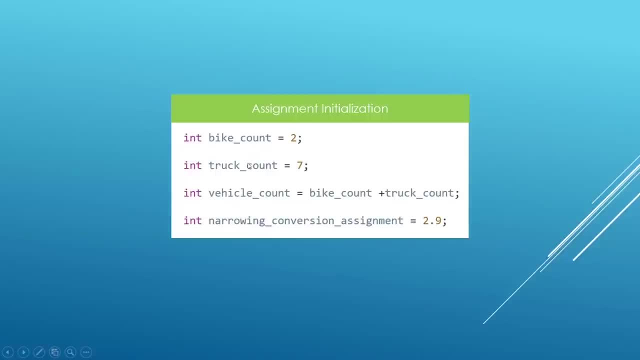 plus, because that's going to be confusing to your compiler, and these are a few rules you really need to be aware of and you're mostly going to be fine. the general form for declaring and initializing your variable is what you see. here you're going to pass the type. 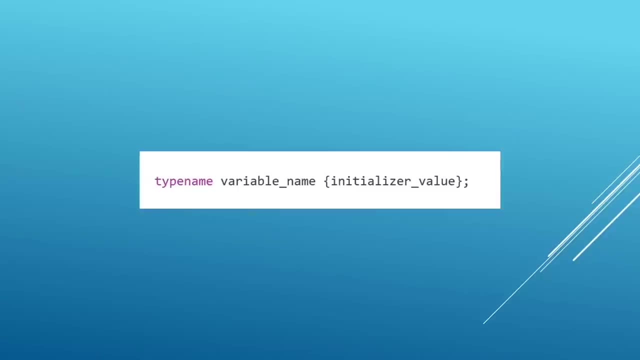 in this case, we have used ant because we are learning about ants. you're going to pass the variable name and you're going to put whatever it is you are initializing your variable with. of course, this is braced initialization because least using curly braces, but you can also use 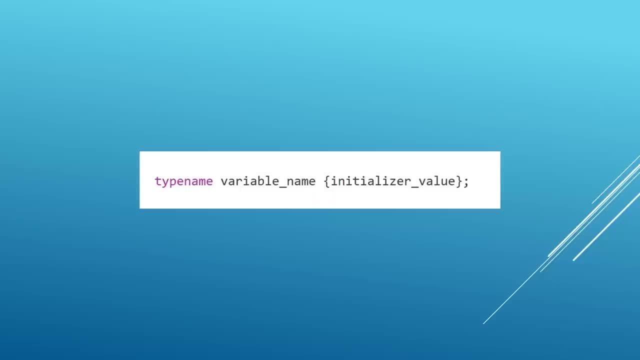 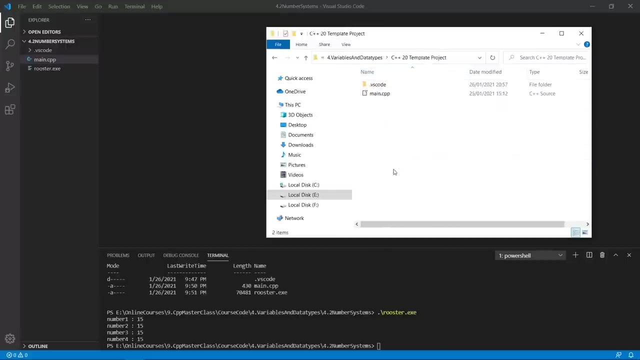 functional initialization or assignment initialization, and it is going to work equally well. okay, now we have enough information to go in visual studio code and play with us. okay, here i am, in my folder for the projects of this chapter. i am going to hop over in my template project. 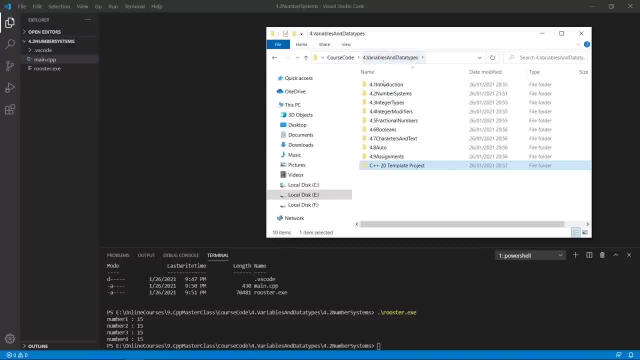 and copy the files that i need. i am going to go up again and go on the project that is called integer types. i am going to go in and paste in my files and i am going to open up this folder in visual studio code. i am going to close the. 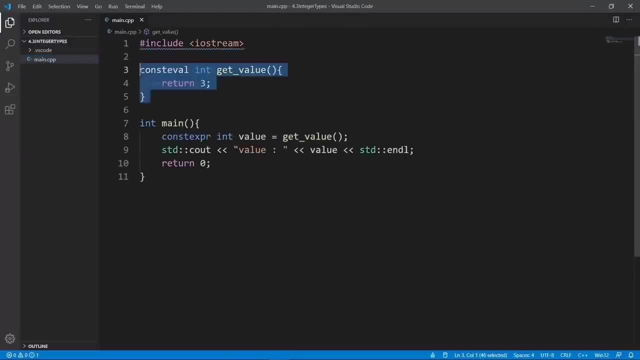 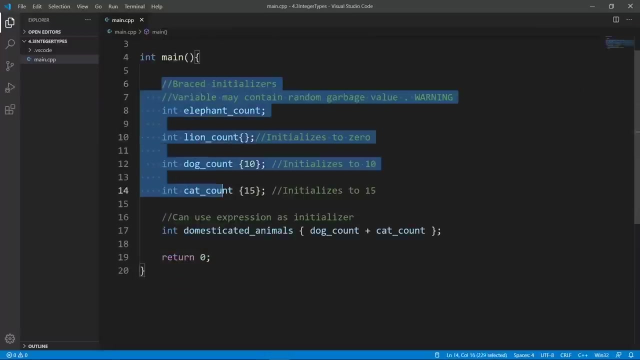 screen here and open my main CPP file, and I am going to do the usual: take out the things we don't need. to save on time, I am going to put in a piece of code that I have lying on my drive and we're going to go through it to save on typing. 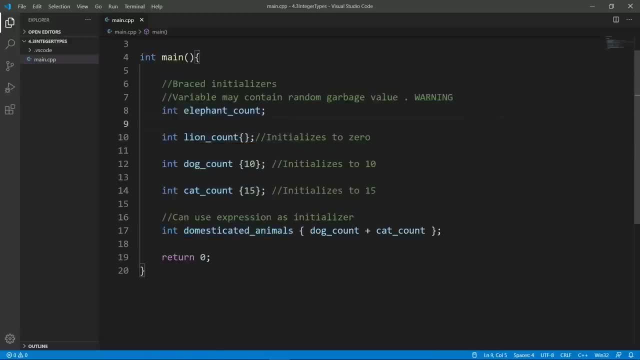 time. I don't want you to suffer watching me type this. the first thing we have is the elephant count. this is a variable that is not initialized, so this is going to contain garbage data. it's not going to contain anything that is useful to us, but some compilers are going to usefully. put in is zero, because that's a logical. 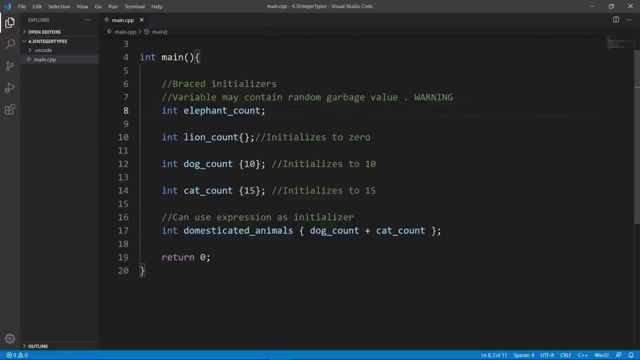 number to put in here if you did it explicitly put a number in here. the second one is using curly braces and this is going to automatically initialize to zero. the third one is going to be explicitly initialized with a 10 and the cat count is going to be initialized with 15. you can try and. 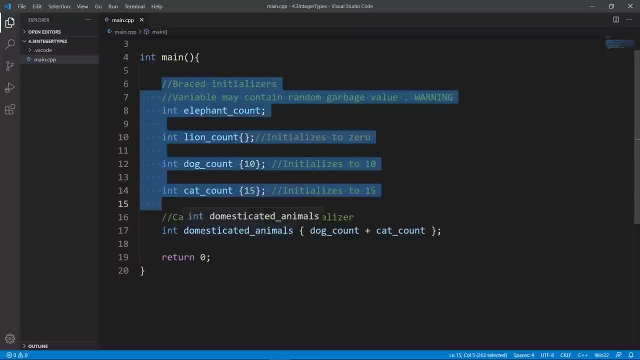 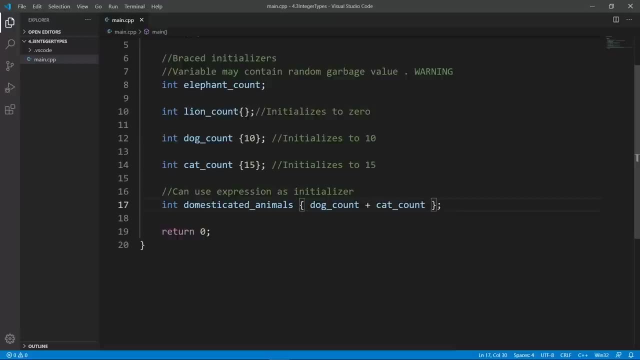 initialize with 15. you can try and initialize with 15. you can try and print this out and see what you come up with after compiling this application. another thing we have seen is that we can do something like this and put an expression into our curly braces, and the value this evaluates to is going to. 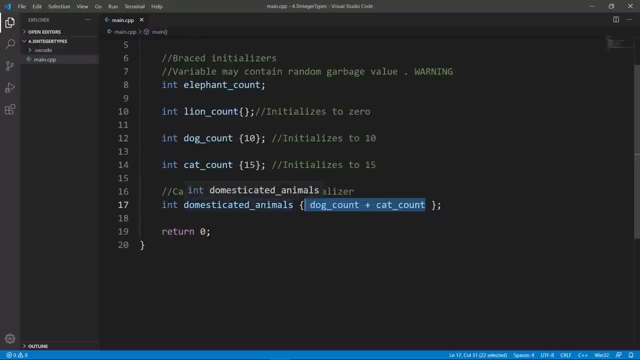 initialize this domesticated animals variable, and now you should know that this is probably going to take four bytes in memory because it is an integer. this is really how C++ works. each fundamental type has a size associated to it most times, so integers is mostly going to be four bytes on your system and we're going to query this a. 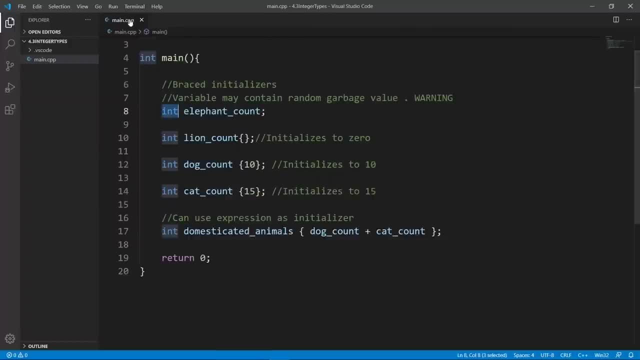 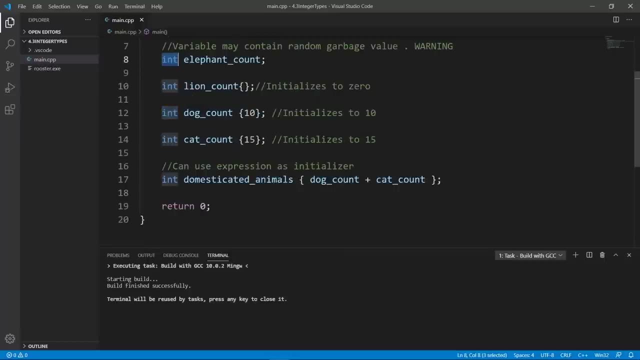 little later in this video. okay, let's try and compile this program and see if it actually works. we're going to start world and you see that the world is successful. another thing we can do is try and use variables we haven't really declared in our program and you can guess what is going to happen. 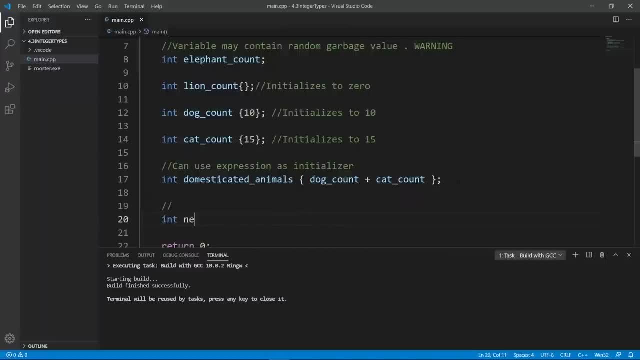 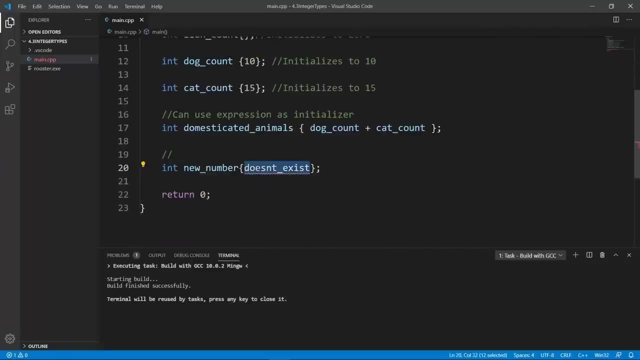 if we try to do and new number, for example, and put in doesn't exist, you know it's a number that doesn't exist. the compiler is not going to know what this is, because we didn't declare a variable called doesn't exist. if you try to compile this, you're going to get a problem. you see that we have a problem. 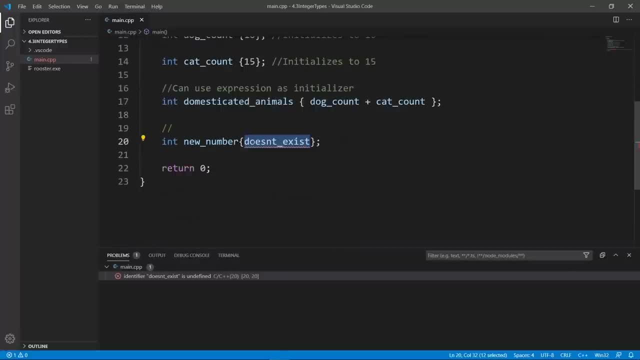 before we even compile. so Visual Studio code is this smart: it can analyze our code before we compile it and give us hints to problems that might come up. and you see here it is saying doesn't exist, isn't defined. so if we try to compile this, we're going to get an error that we expect. it's going to say doesn't exist. 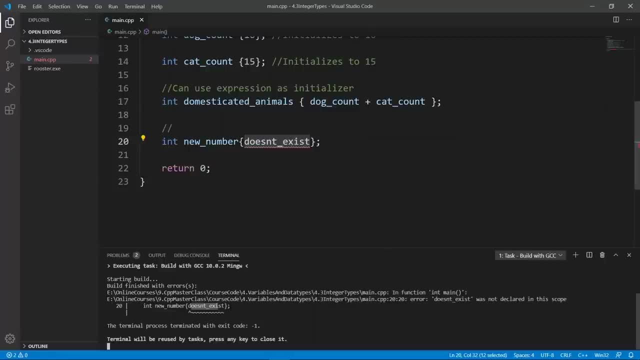 doesn't really exist. I don't know what that is, so you shouldn't really do that. you shouldn't try to use variables you haven't declared. this is braced initialization. we can also do functional initialization, as we have seen. okay, another thing we can do is store a fractional number in an initialization. 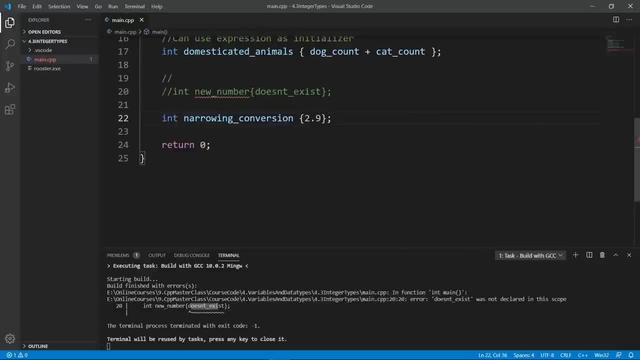 variable and we're going to see what this does. we're going to try and compile this code. you see, we have a 2.9. we're trying to store this in an integer. if we try to compile this, let's try and use GCC. let's clear this. let's bring up a. 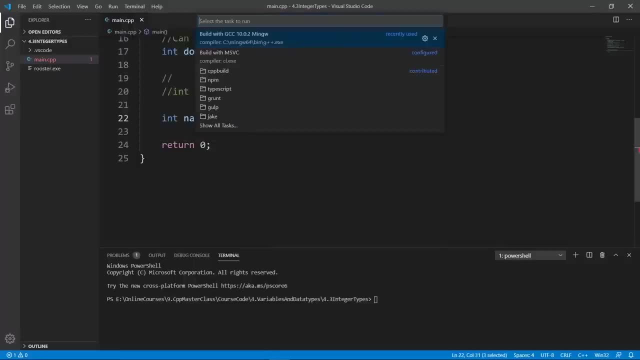 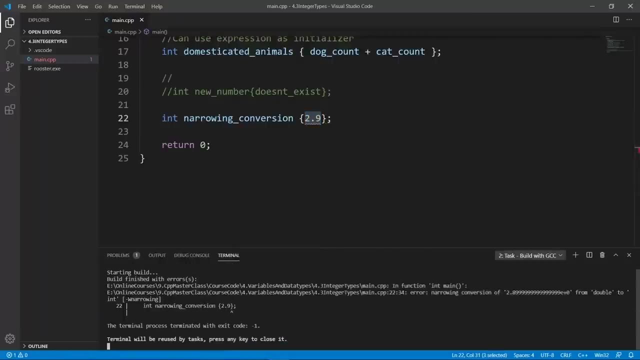 terminal and try to build this. we're going to try and run our GCC compiler on this program. it is going to say arrow narrowing conversion of 2.899 from double to integer. C++ 20 isn't even going to allow this. so this is a good thing, because you might think. 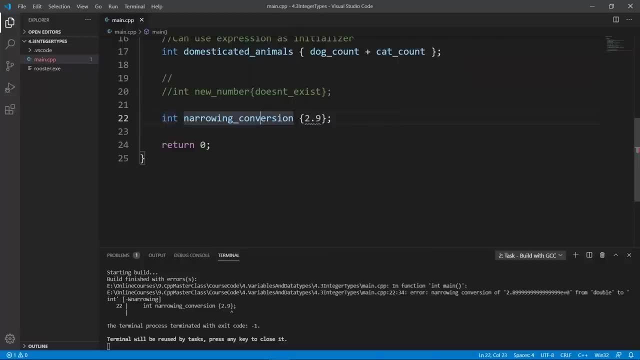 that you have a 2.9 and some compilers are going to chop this off and to store a 2 instead. so this is one of the safe things about this way of doing things. so I am going to comment this out, because otherwise our program wouldn't compile. 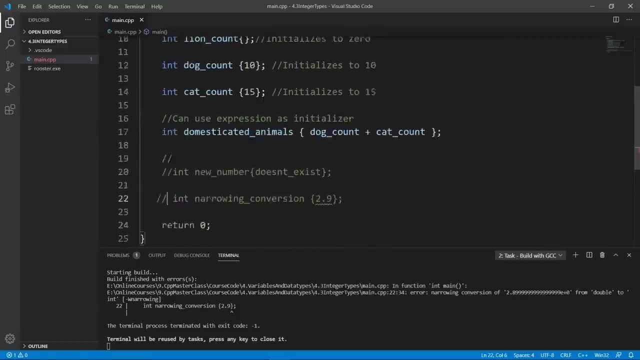 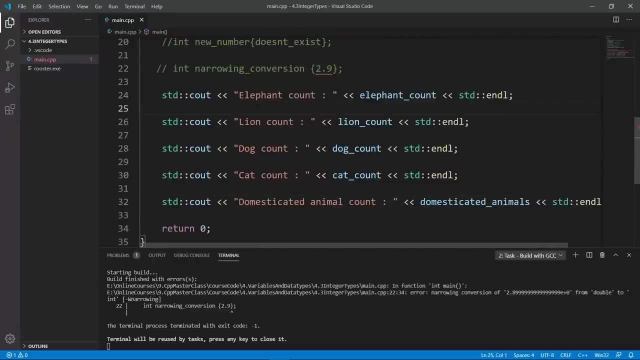 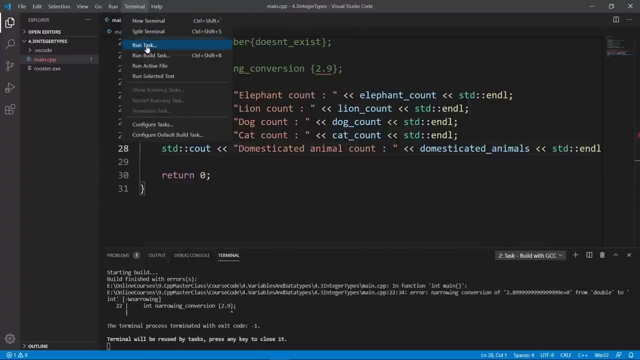 now that we know how to use these things, we can try to print the values in here. okay, I am going to put in a piece of code I have lying around on my drive. I am going to remove these spaces inside because it is annoying. let's do this. and if we try and build this program, it 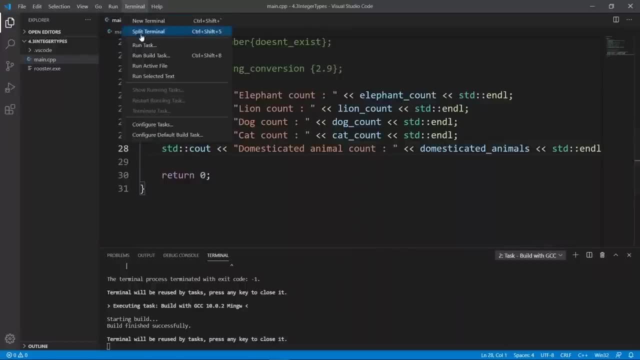 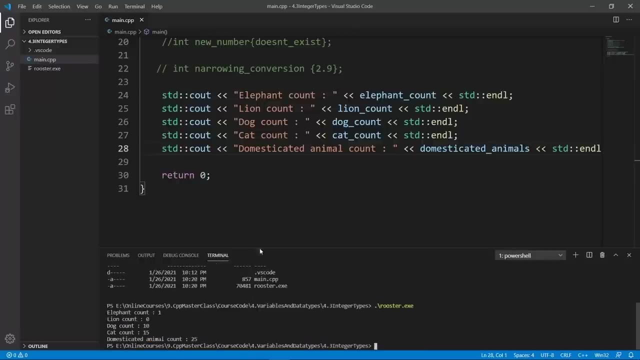 should compile successfully and if we run it, we should see our numbers. we're going to go in our terminal here and do there and we're going to run rooster and we're going to see elephant. count is one, because this is a garbage value, so it 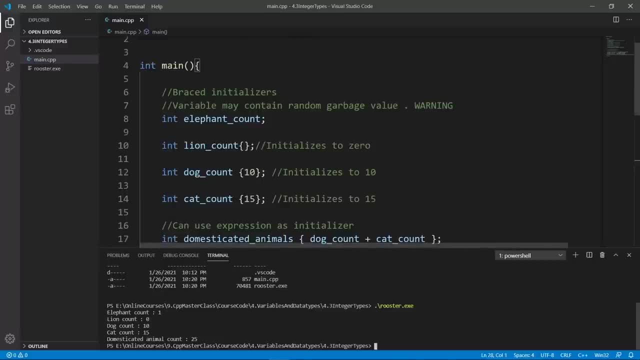 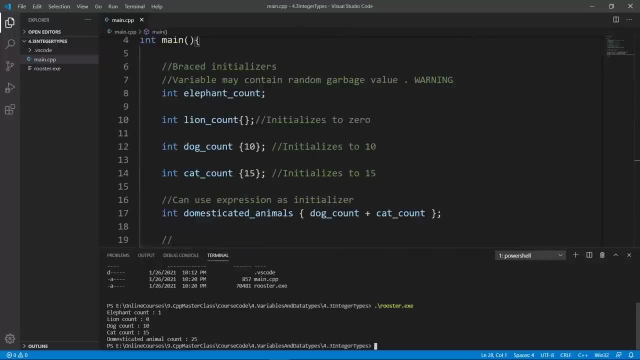 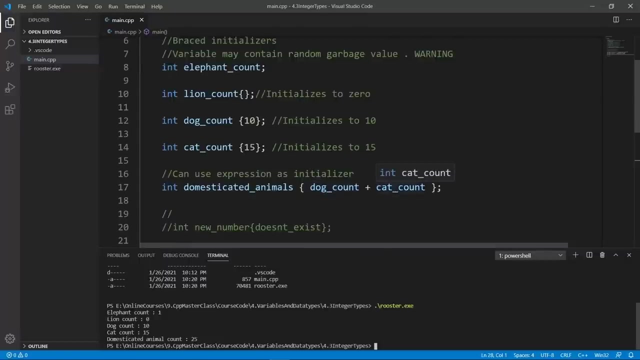 could really be anything. lion account should be zero, should be 10, cat count should be 15. it is what we have and domesticated animal count is 25 because we have double count and we add that to cat count and we're going to end up with 25. this is what we expect now that we know how to work with. 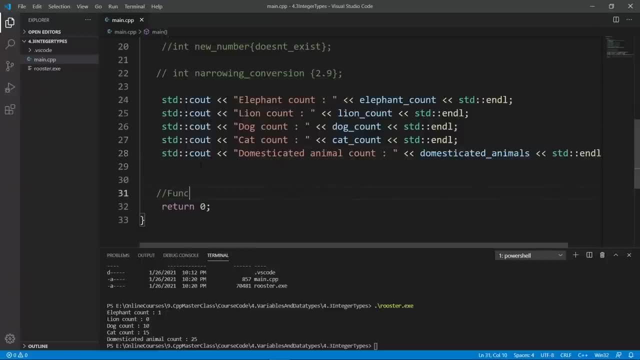 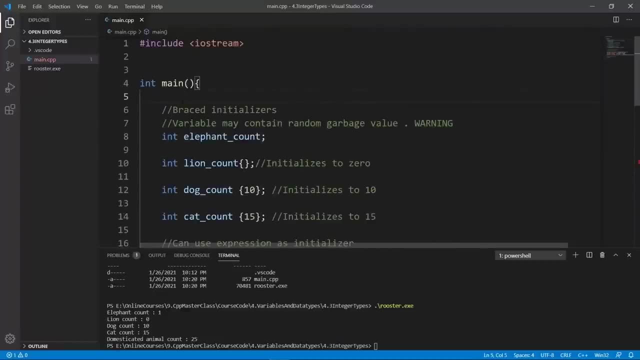 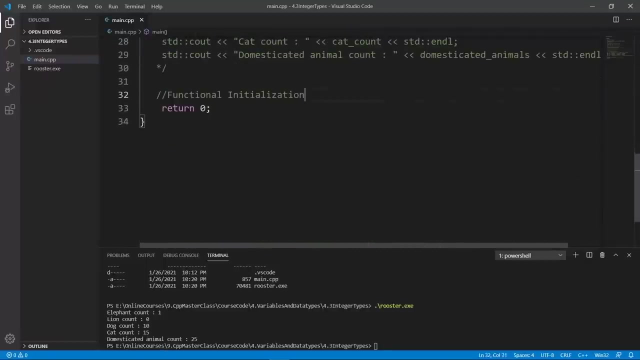 this. we can also try and play with functional initialization before I put in my code. I am going to comment all this out because I don't want this to disturb us. we work with our functional initialization code, so i am going to comment all this out and go all the way down. 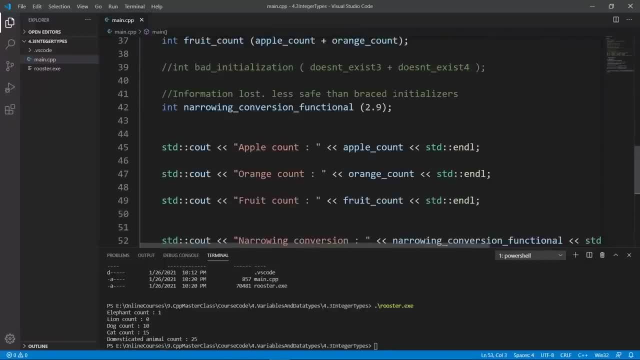 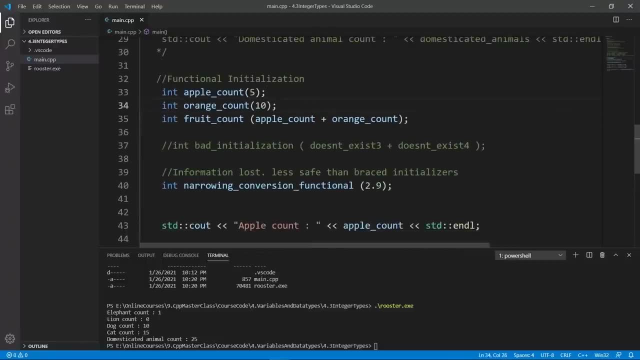 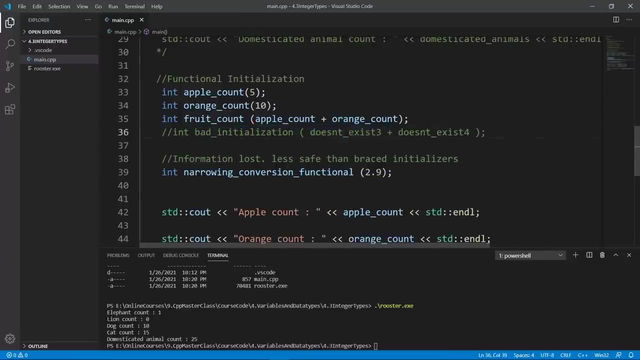 and put in my code for functional initialization and you see, here we have a variable called apple, we initialize this to five, we have orange count, which is 10, we have fruit count and we have a bad initialization. that is not going to work. it doesn't exist three and doesn't exist four, don't. 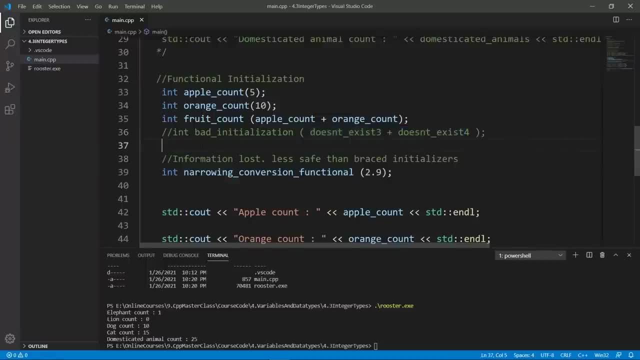 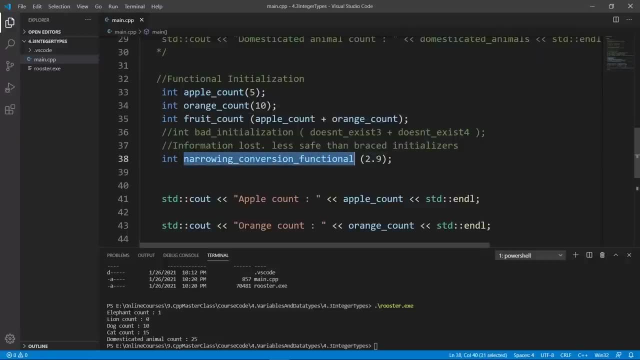 really exist so. so this is going to give us a compiler error and if we do something like we do, a narrowing conversion functional here, this is mostly going to compile and this is going to chop off data and store a two instead of the 2.9. this is something you should really be aware of, and 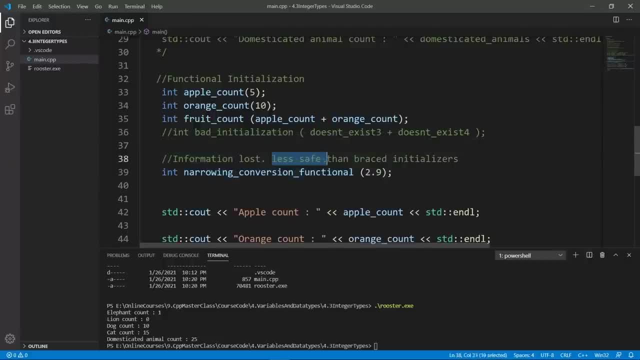 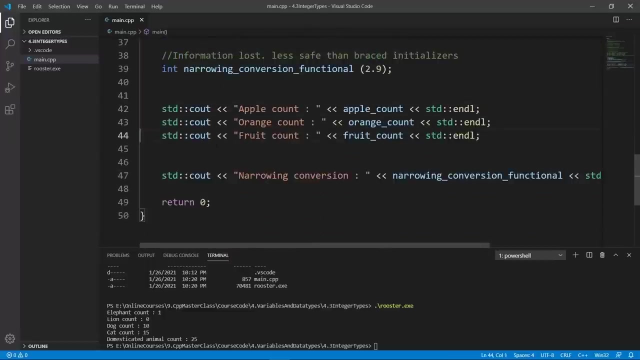 you see, the comment here says: information lost. this is less safe than braced initializer, because braced initializer is going to give you a compiler error if you try to do this, and that's a good thing. so we also try and print these out. so i am going to tidy this up a little bit and i am going to try and compile this piece. 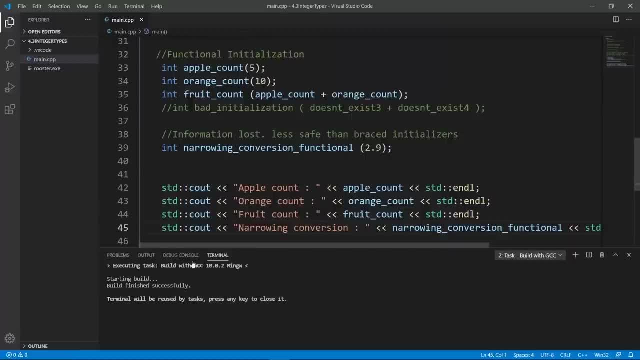 of code, run task and world. with gcc, the world is going to pass through without a problem. and if we do clear and run rooster, we're going to see apple count is five, which is what we have in here. orange count is going to be 10. 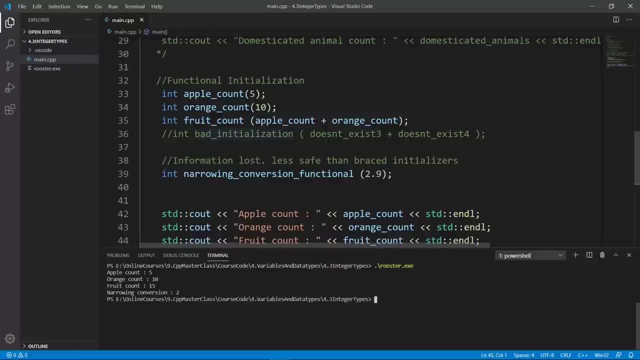 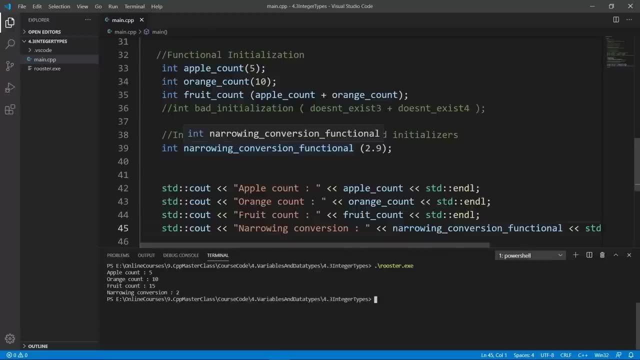 so, So, this is right. Fruit count is going to be 15, because it is 5 plus 10.. And what is really worrying is that narrowing conversion is 2, but we didn't store in a 2. We stored in a 2.9.. 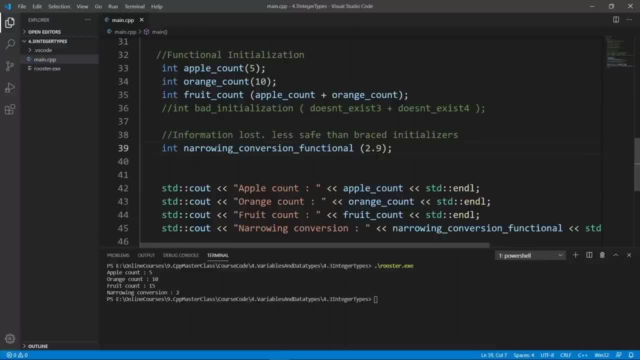 And because an integer can really store 4 bytes. 2.9 is more than 4 bytes And it is going to store what it can And it is going to chop off this 2.9 and only store in a 2.. 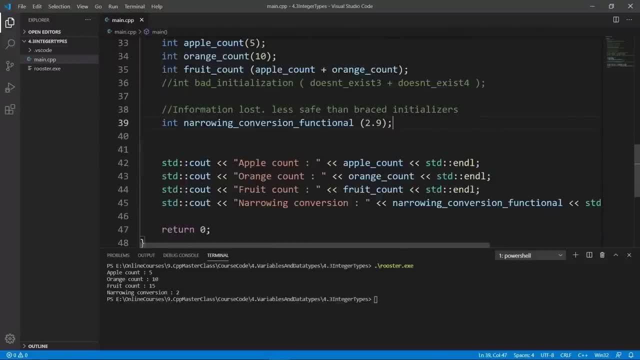 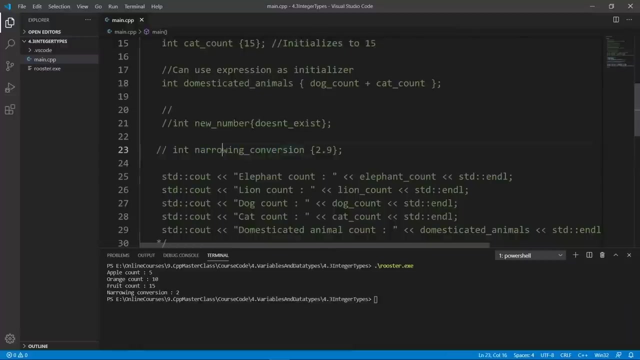 So this is really something you should be aware of. Sometimes this is going to cause problems in your program And really, really, if you are trying to store fractional numbers in an integer, please use a braced initialization form, because the compiler is going to stop you from doing this if you try. 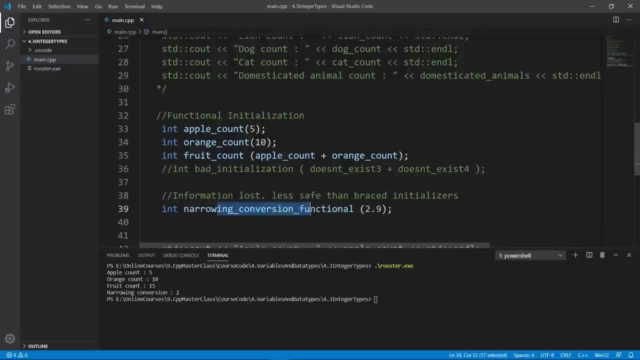 Okay, so this is really the difference between functional notation and braced initializer notation. Functional notation is not going to give you an error if you try to store something that can't really fit in a net. It is going to silently chop it off and put in whatever it can. 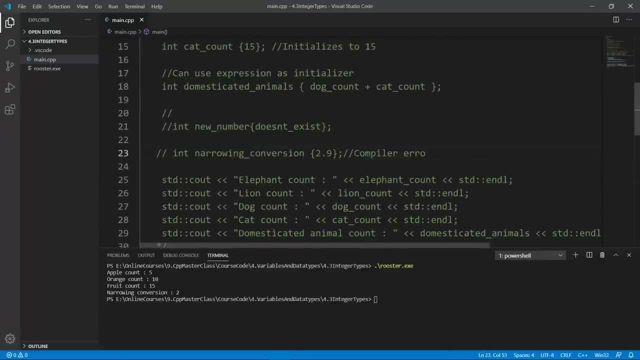 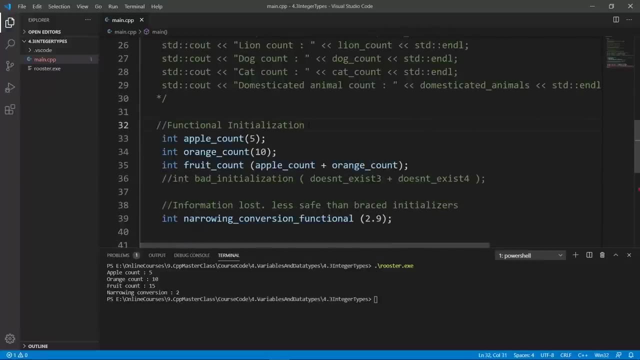 And braced initializer is going to give you a compiler error. So this is the difference between these two. Okay, I am going to comment this out as well And I am going to put the starting comment here And I am going to go down and show you. 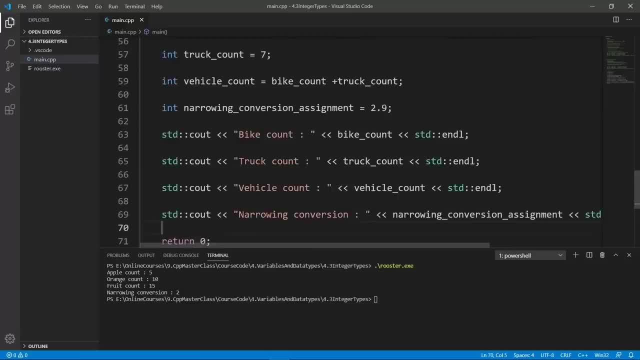 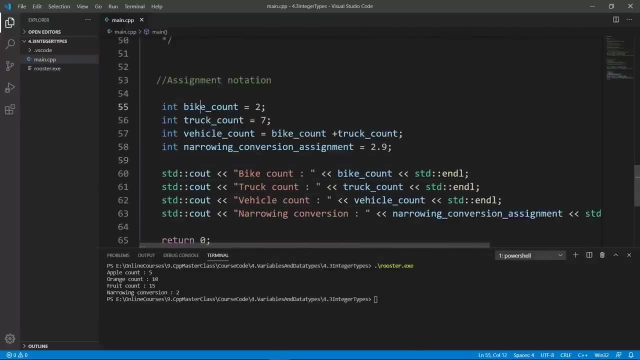 that you can do assignment initialization as well. I am going to put in my code here, because I don't want to type it really, And I am going to print all this out. And we have a bike account variable that we initialize using the assignment notation. 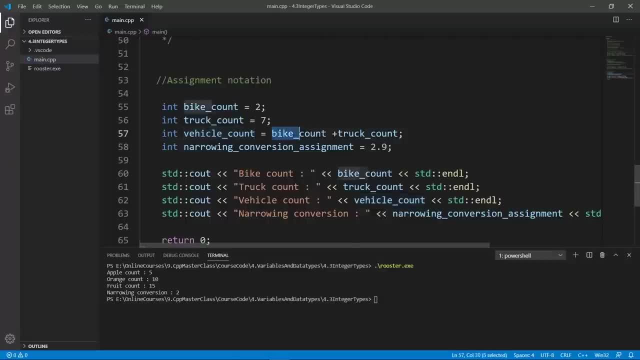 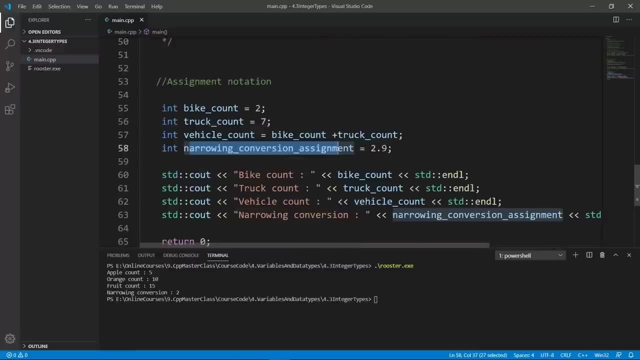 Track count is going to be seven. Fake account is going to be bike count plus track count And we're going to be narrowing conversion here And we're going to see if this actually works. We're going to try and build this. We're going to run the task to build with GCC. 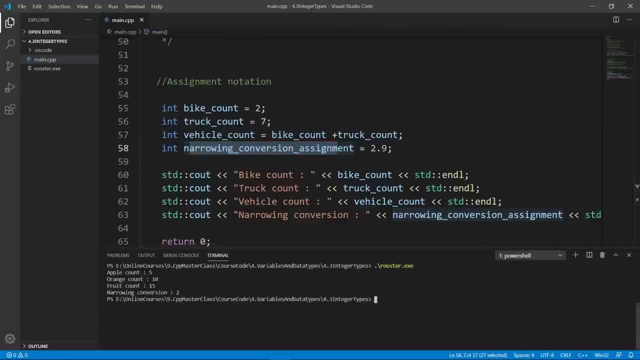 It is going to pass through. You can guess what we're going to see if we run the program. Bike account is two, Track count is seven, which is what we expect. Fake account is nine And the narrowing conversion is also chopping off. 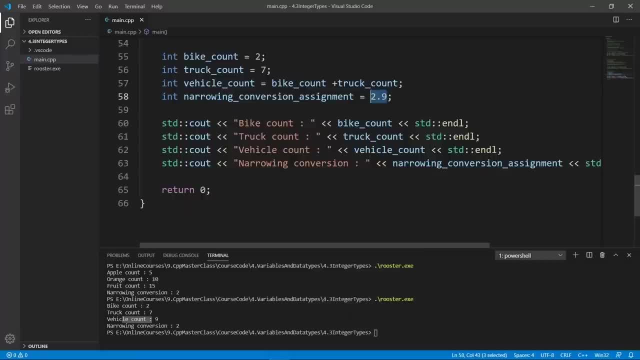 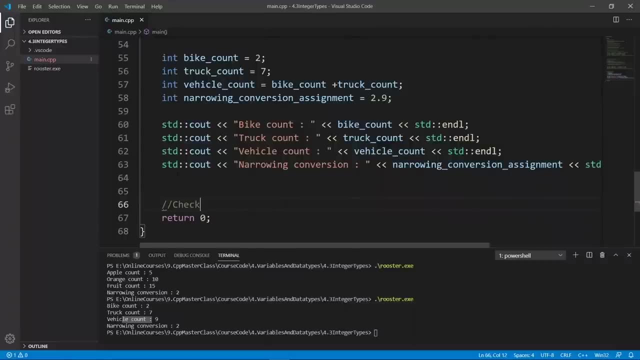 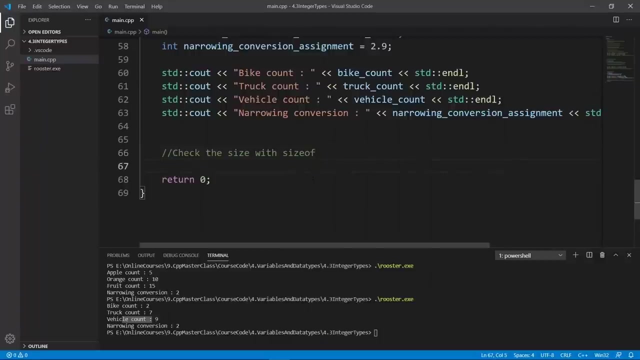 what we have here. So this is something you need to be careful about. Another thing I want you to see is that you can check the size of your variables in memory. So we're going to check the size with size of, And I am going to put in a piece of code. 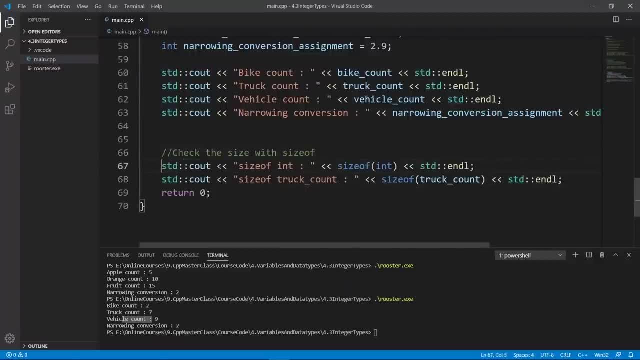 to really play with this. I don't want to type all this, because it's really self-explanatory by now. We're going to print size of int And inside we're going to say size of int, And this is going to give us how much memory. 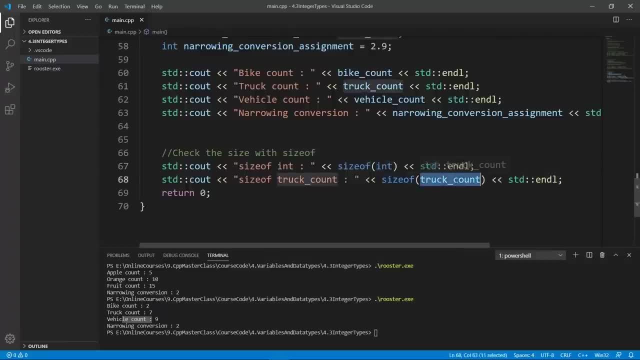 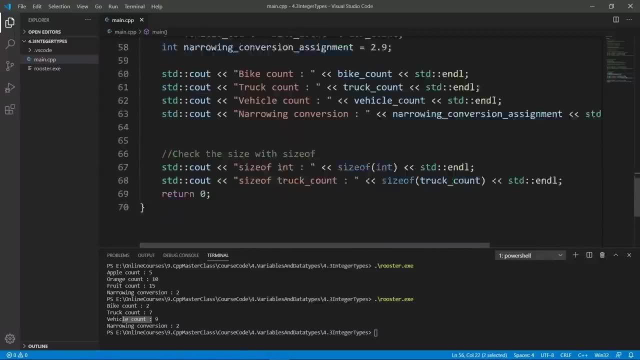 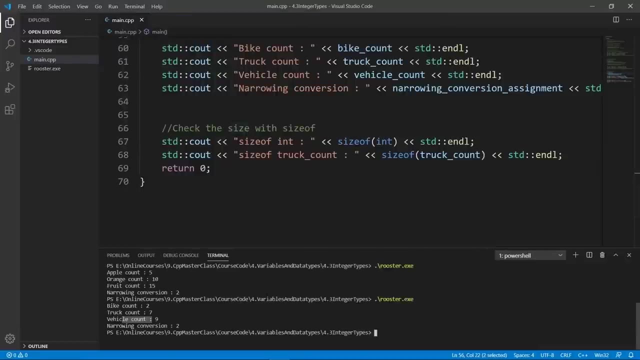 is really occupied by an int And we can use this form here by passing in a variable name. Track count is a variable we have declared and initialized here. So if we build this program, let's do that with GCC. the build is going to pass through. 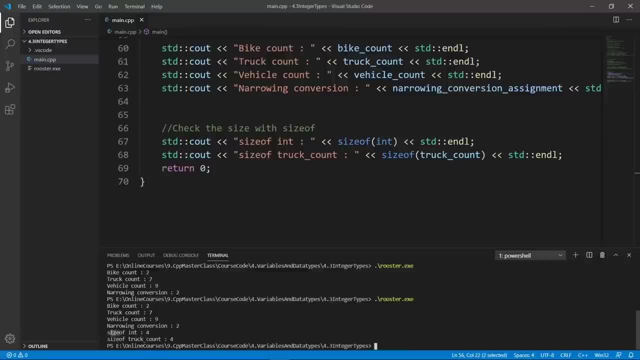 And if we run rooster, we're going to see that the size of int is four. You're going to see that this is in bytes And size of track count is four as well, because track count is also an integer. So these are all little tools you can really use. 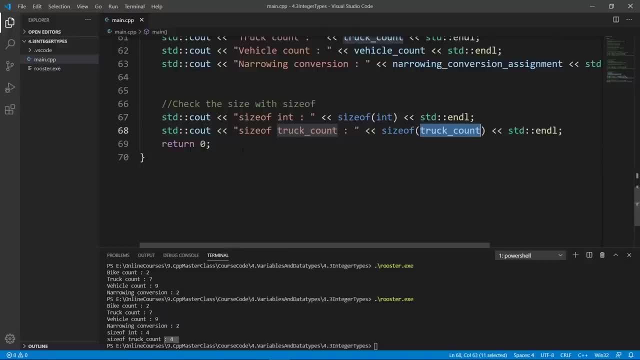 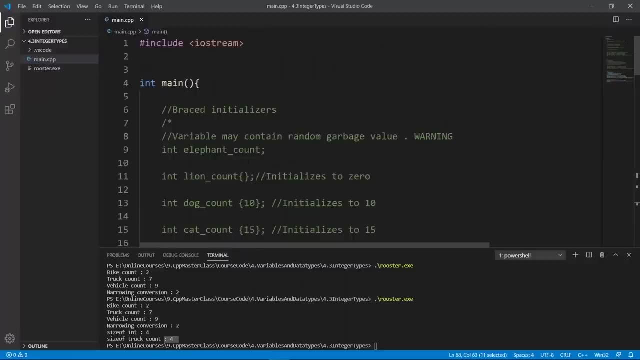 to know how much memory is really being used and occupied by your program, And this is really all we say. So to do in this lecture, to learn as much as we can about integers. Integers occupy four bytes in memory for the most part. 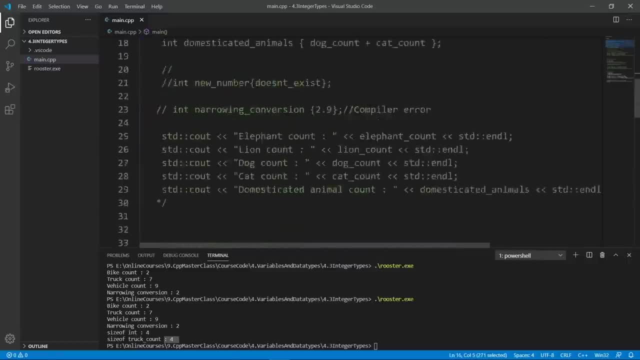 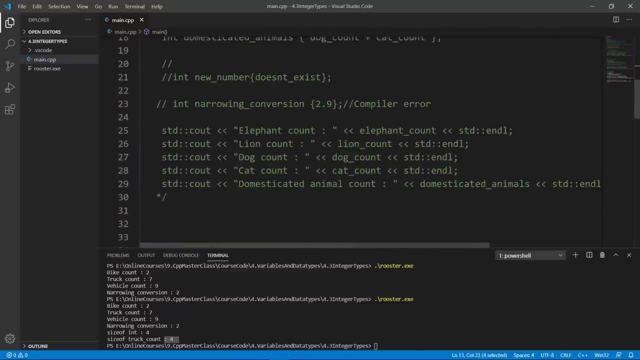 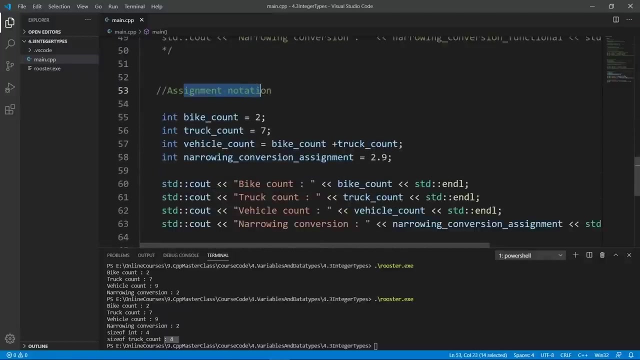 And we have seen different ways we can initialize our integer variables. We can use breast initializers. which is going to use curly braces? We can do functional initialization using parentheses like this. We can also do assignment notation using a from like this: And we can use size of to check. 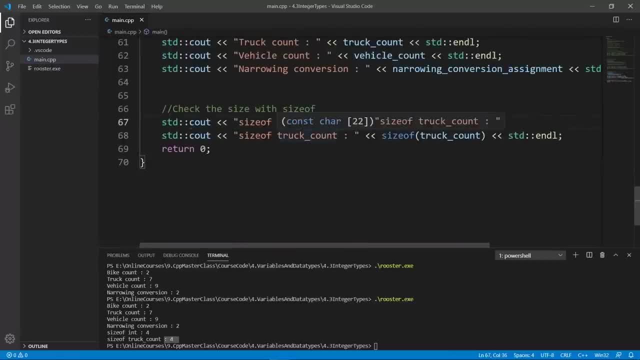 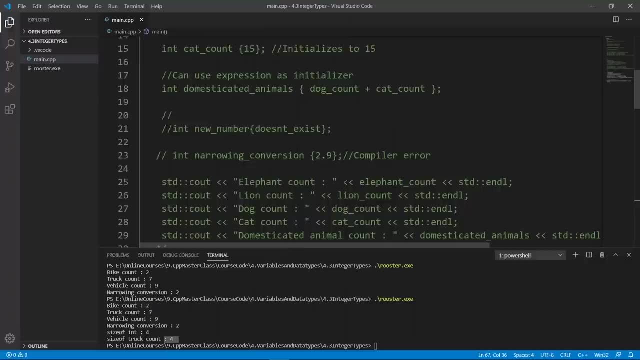 the size of our integer variables. I have to say that these kinds of initialization also work on other variables, but we took the chance to introduce all these concepts using integers. This is really all we set out to do in this lecture. I hope you found it interesting. 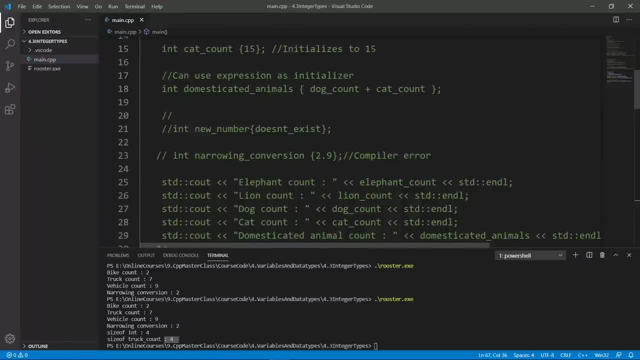 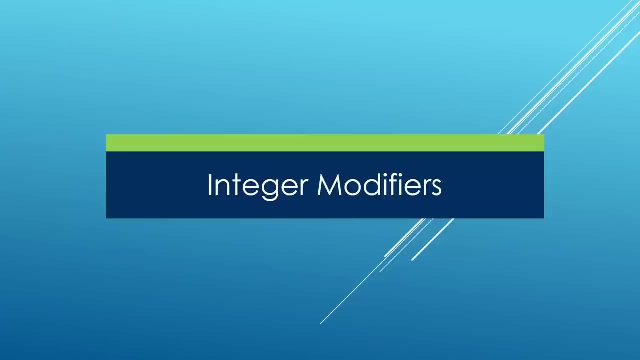 We are going to stop here in this lecture. In the next one we're going to start and learn about integer modifiers. Go ahead and finish up here and meet me there. In this lecture, we're going to learn about integer modifiers, And these are little things you can sprinkle. 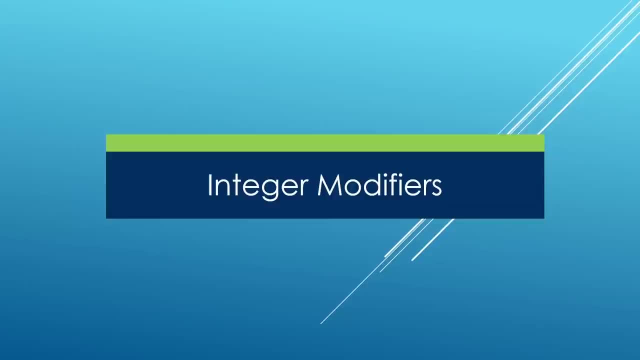 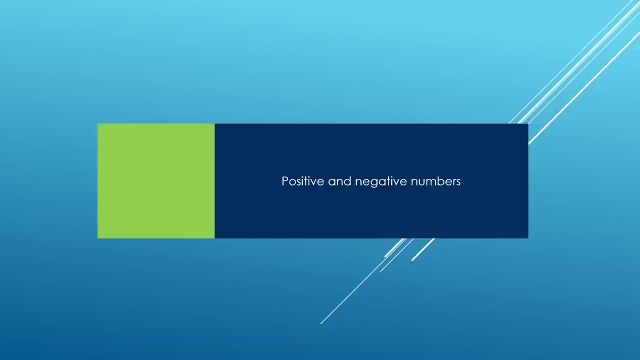 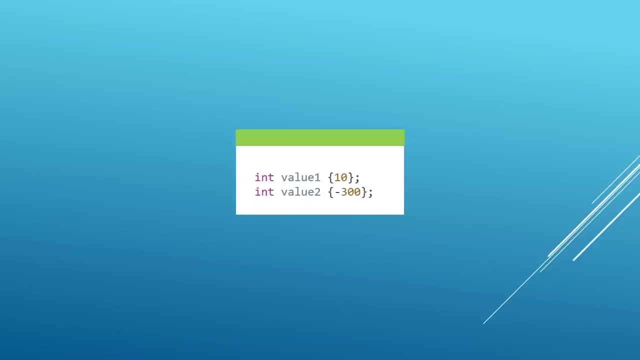 around your integer types to modify their behavior a little bit. But before we dive deep into this, let's talk about how we can store positive or negative numbers in integers. And we can do something like this: If we put a 10 inside our value, one variable, 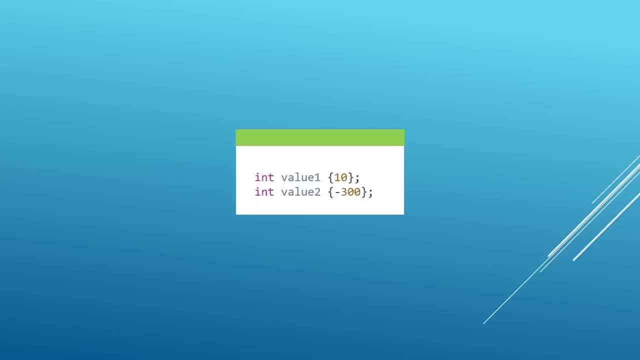 which is an integer. it's going to work. We can also put in a negative number, like minus three. We can also put in a negative number like minus three, And it is going to work. So what's the magic here? 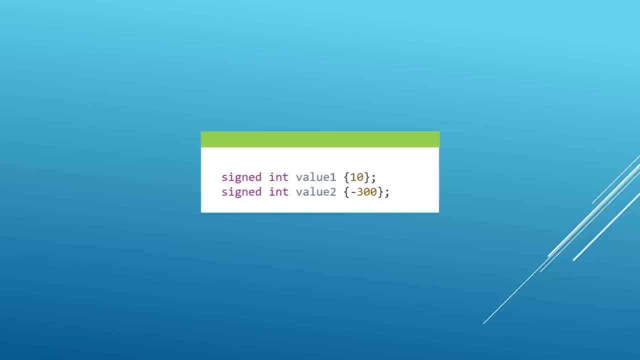 Well, this is signed by default And this is a modifier we can apply to our variable to signal that we have the possibility to store in negative or positive numbers, And it is going to work If you only want to store positive numbers in your int variables. 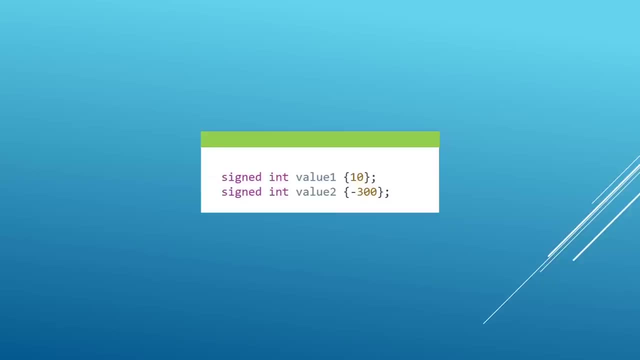 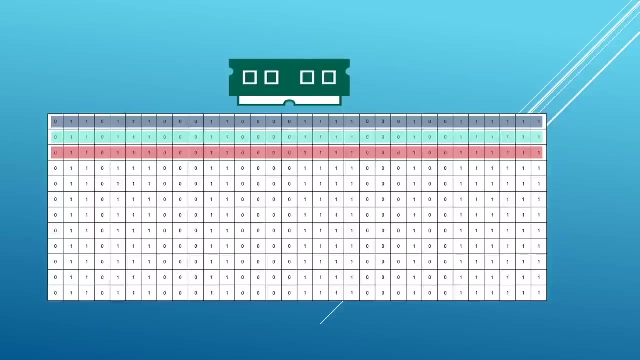 you can use another modifier called unsigned, And if you put in a negative number, you're going to get a compiler error. We're going to see how this works in a minute. Okay, regardless of whether your integer variables are unsigned or signed. 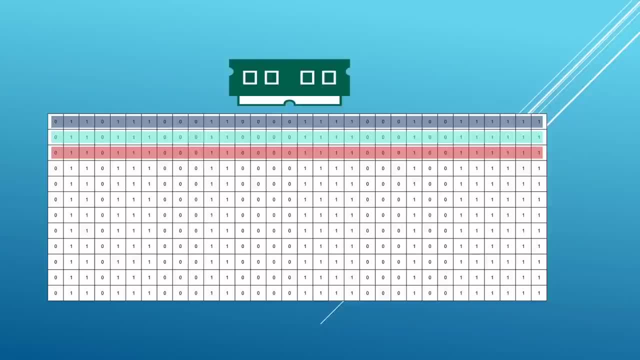 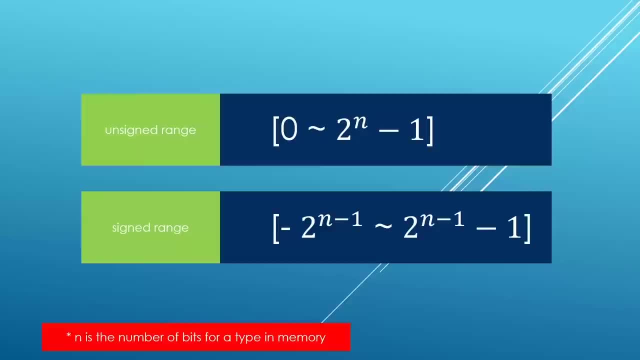 they are going to still occupy four bytes in memory. So this is how it's going to look in memory, And here is a simple formula we can use to come up with the range of values we can store in our int values if they are unsigned or signed. 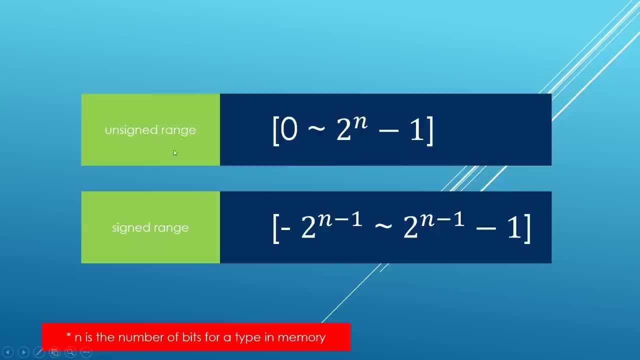 If the number is unsigned, you can use this unsigned range, the range formula, and plug in the number of bits you have in your data type. If you are using a signed integer, this is what you're going to use, And here is a simple example. 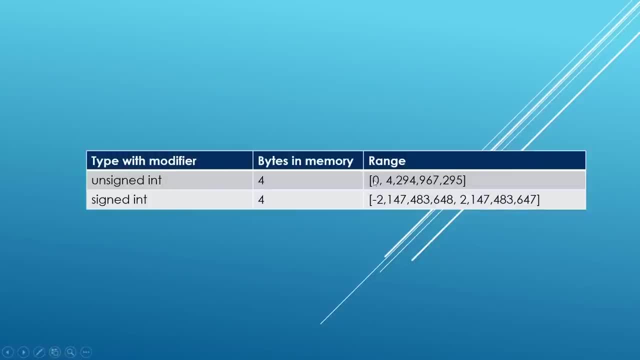 For example, if we have an unsigned int, this is the range of values we can store. We can basically go from zero all the way to 4 billion. If the number is signed, the range is going to basically be divided into half. 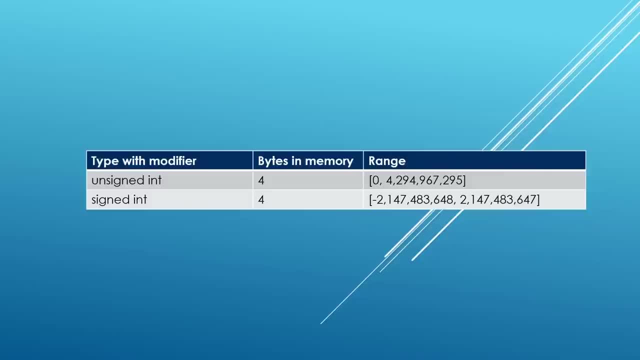 The half is going to go on the left and store negative numbers And the other half is going to go to the right and store positive numbers, And you can see that we can basically go from minus 2 billion to 2 billion if the number is signed. 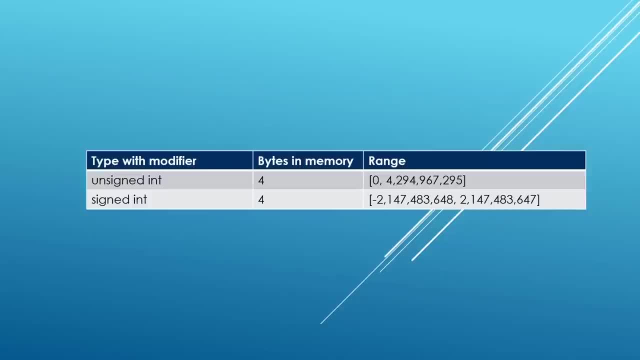 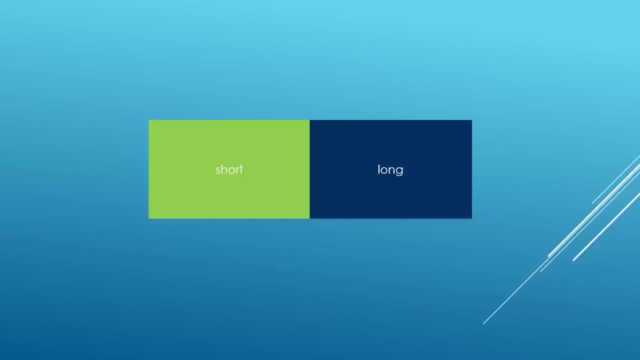 Okay, by now we have seen two modifiers- unsigned and signed- but there are others. For example, you can flag your integer types as short or long. What does this do? Well, this is a table that I put together to try and come up with all the components. 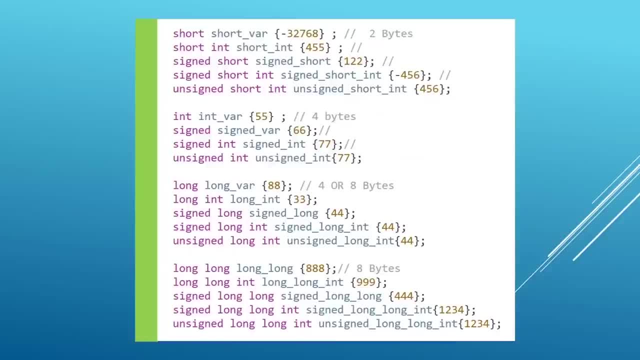 Well, this is a table that I put together to try and come up with all the components. Well, this is a table that I put together to try and come up with all the components, To explore what combinations you can come up with if you have a short variable. 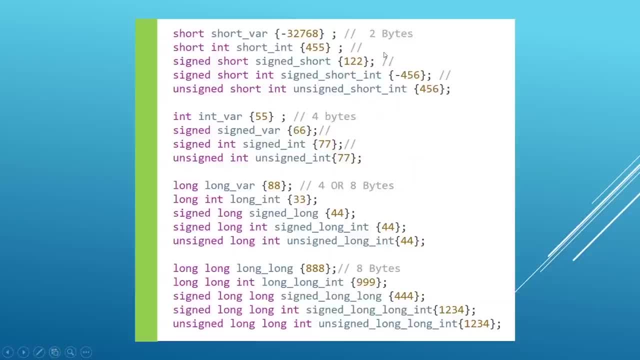 it is going to be two bytes in memory. This is the modification that this modifier does to your type. If you have short, and it's going to be two bytes. If you have signed short, and it's going to be two bytes. if you have unsigned short, and it's going to be two bytes. 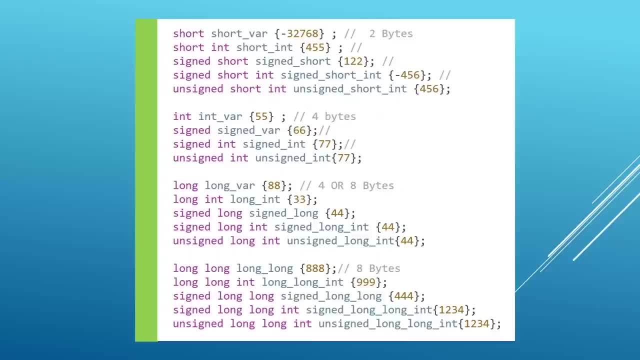 You can see that theд effect of short is really shortening the original size in memory for whatever type you want. applied this on, this is really working on an editor. even if we don't specify int here, for example, short, short, here it's going to implicitly be int. that's why we have two bytes, because it's 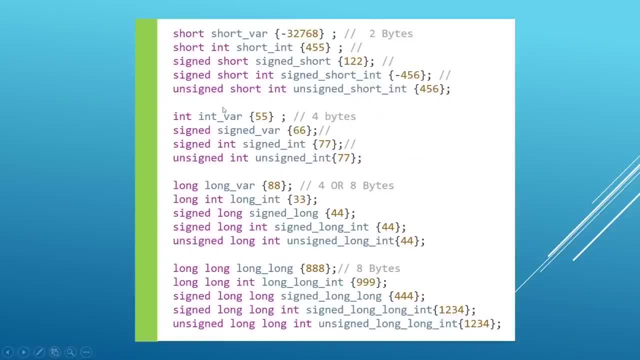 basically an int that we have split in two. here in the second column we have int, which is going to be four bytes if it is assigned, and it's going to be four bytes. this is really the sizes you're going to come up with if you use these combinations of modifiers on your integer times. one thing i 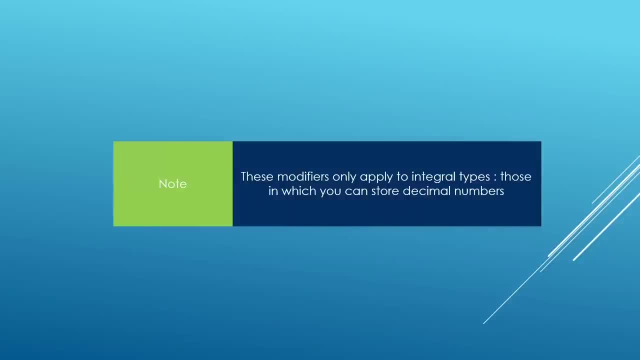 really want you to be careful about is that these modifiers only work for integral types, so they work for data types in which you can store decimal or whole numbers. you can't use this on types in which you can store fractional numbers like 2.9. that's going to give you a compiler error now that. 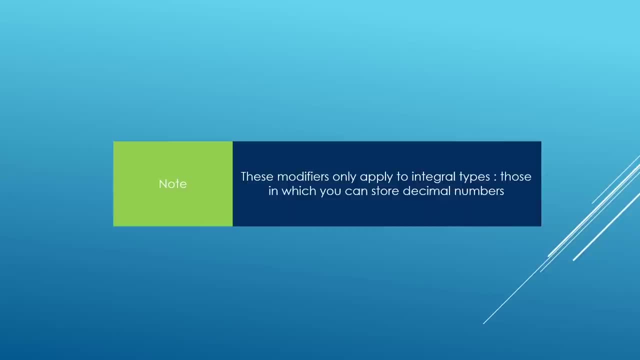 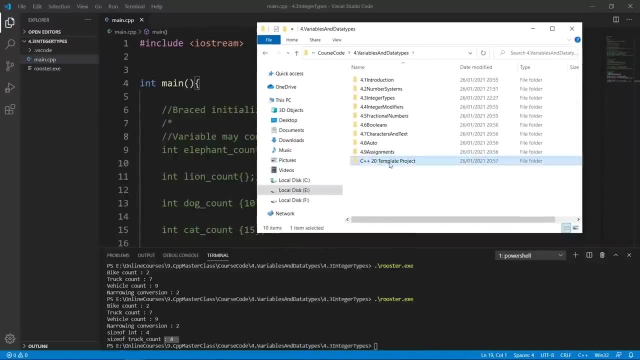 you have an idea about this. why don't we go in visual studio code and actually play with us? okay, here we are, in our folder that contains our projects. we're going to do the usual and copy the files from our template project and we're going to put those files in our integer modifiers project here. 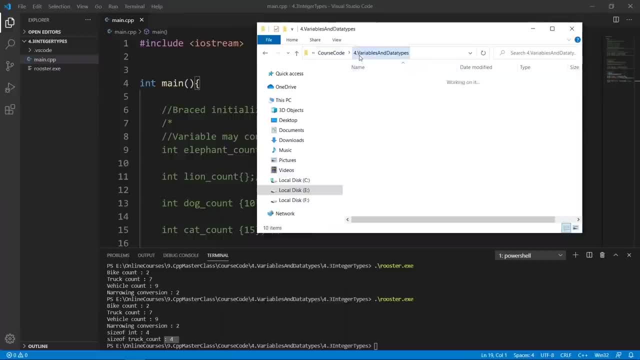 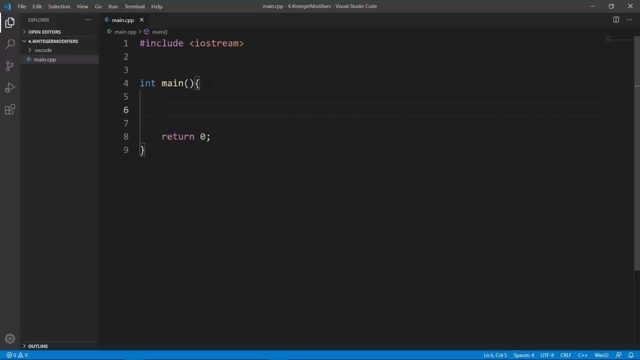 let's open it up and paste in the files we're going to go up again and we're going to open this up in visual studio code. the first thing i want to play with is storing positive and negative numbers in our integer types. so we're going to say int value one and we're going to store. 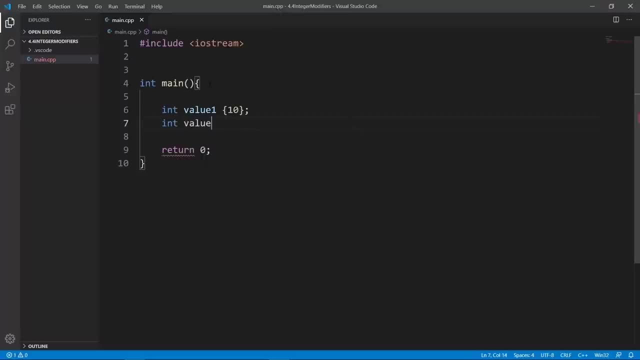 in a 10, for example, and we're going to do int value two and we're going to put in a minus 300. i think this is what we had. you know a slide, so we're going to keep this, if you try to print this out. so we're going to say value one and we're going to say value two, and we're going to try. 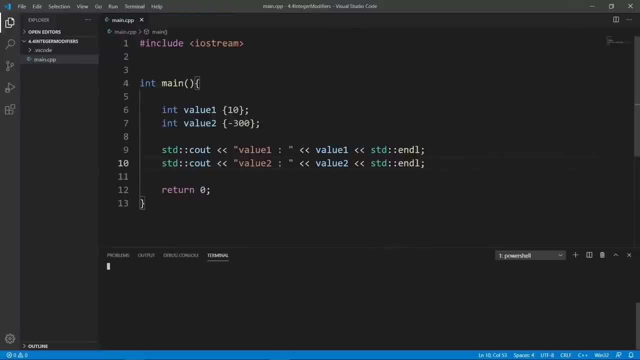 and build this. so we're going to open our terminal so that we can play with it right away and we're going to run the task to build with gcc. the world is going to be successful if we run our program. we're going to see that it's going to say value one is 10 and value two is. 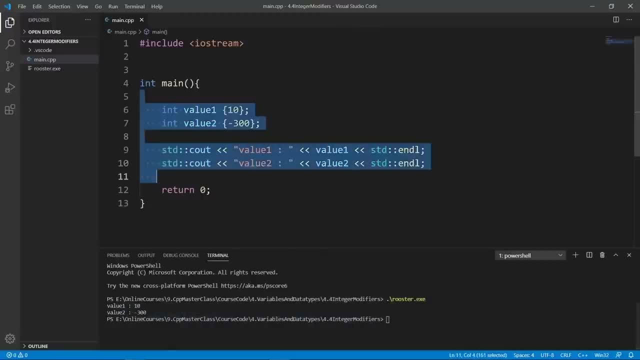 minus 300. this is really cool. we can store positive numbers and negative numbers in our int types and this is going to occupy four bytes in memory. we can prove this by printing the size of value one and value two. let's do that, so we're going to say size of. 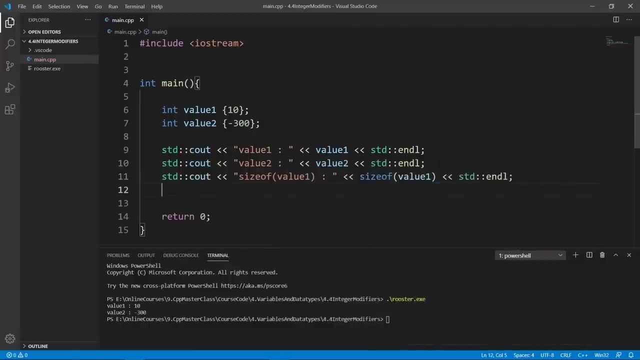 value one is size of value one. we can also do it for value two, size of value two, and it's going to be size of value two, std. and yeah, if we build this again, we're going to run the task to build with gcc and we run our application. it's going to say four bytes. so it doesn't really matter if we store. 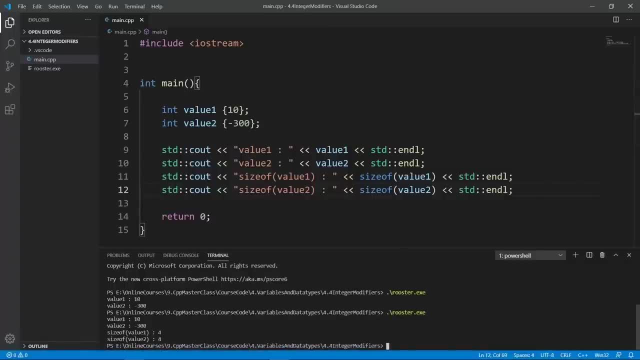 in a positive number or a negative number. it's going to be four bytes. this is the point i want to make here. another thing you can do is actually make it very clear that you have signed numbers in here and you can use the signed integer modifier here. so this is going to give us the same result, and if we try, 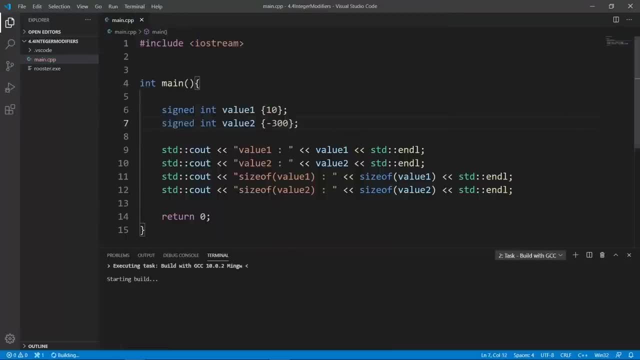 to build again. run the test world. with gcc, the world is going to be successful. if we run the program, we're going to get the same result. so if you don't put assigned or if you put it here, it's going to be exactly the same result. that's what we're going to do here. so we're going to run the. 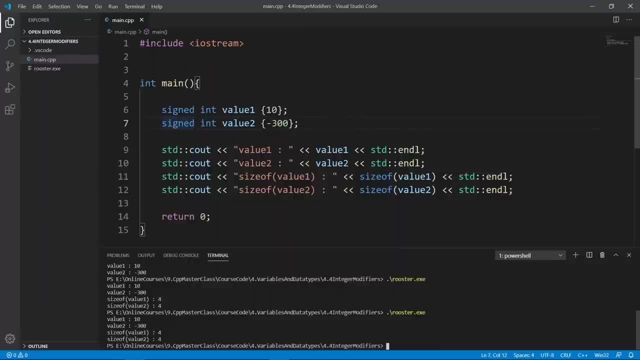 same thing. another thing you can do is make it very clear that you want to store positive numbers in your variables. we can do that by using the unsigned integer modifier. so we're going to say unsigned and value 3, for example, and we're going to put in a 4. this is going to be fine. but if you 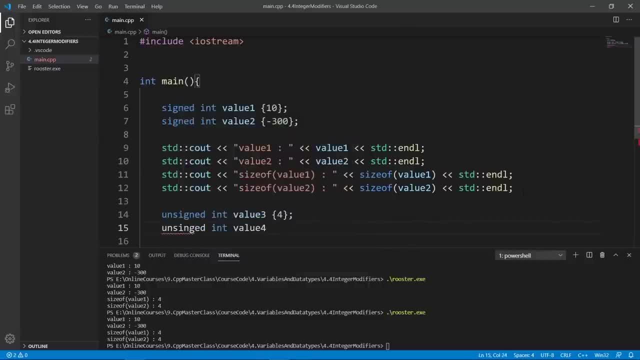 do unsigned and value 4 and put in a minus 5, for example. this is going to give you a compiler error because you say this is unsigned and this really means that you want to store in only positive numbers, but you are trying to put in a negative number. if you're trying to build this, let's try. 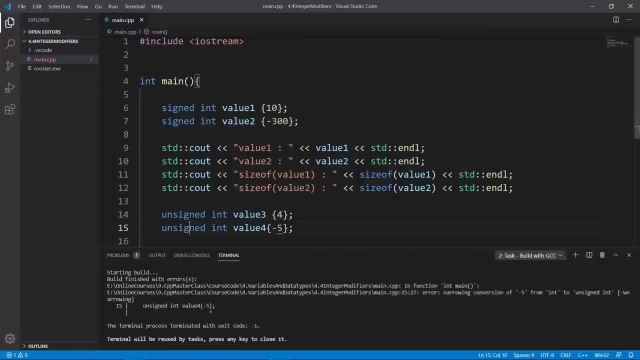 this. we're going to run the task to build with gcc. we are going to get a compiler arrow saying conversion from minus 5 to end this not allowed. you're going to get a compiler error. your program is not going to compile, so this is a compiler error. let's say this here and this is really all i had to share about these signed and. 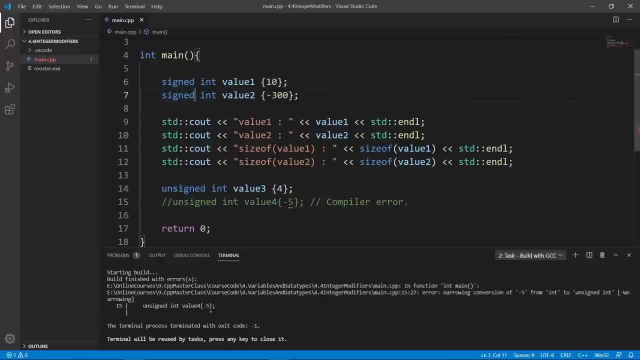 unsigned modifiers. signed is going to mean that you can store negative and positive numbers. unsigned is going to mean that you can only put in positive numbers and if you try to put in a negative number, you're going to get a compiler error. now that this is commented out, if you try to run the test. 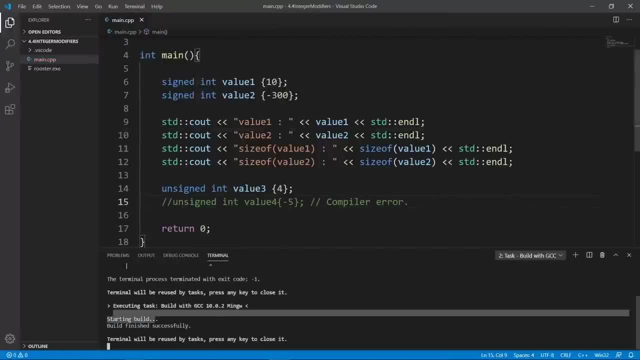 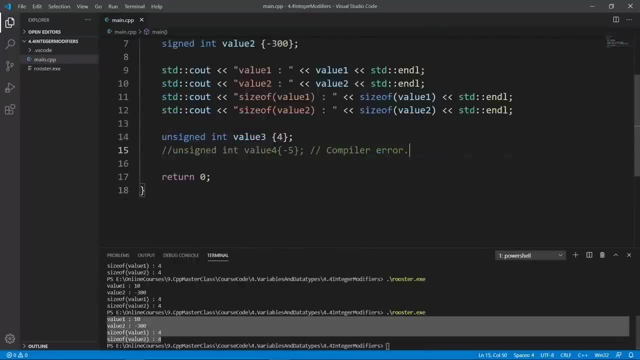 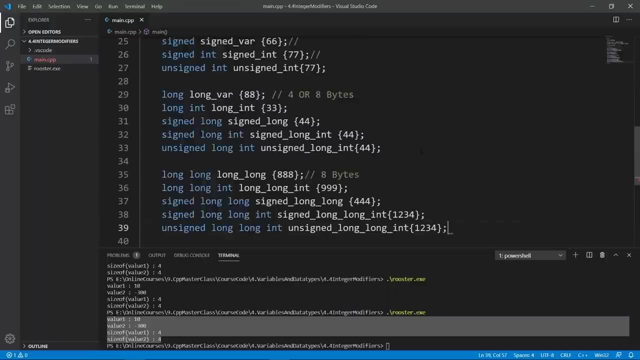 to world. with gcc, the world is going to be good and we will be able to run our program, and it's going to do whatever it was doing before, as we see here. we also saw that we could use the short and long modifiers, and we're going to put a piece of code here that is going to allow us. 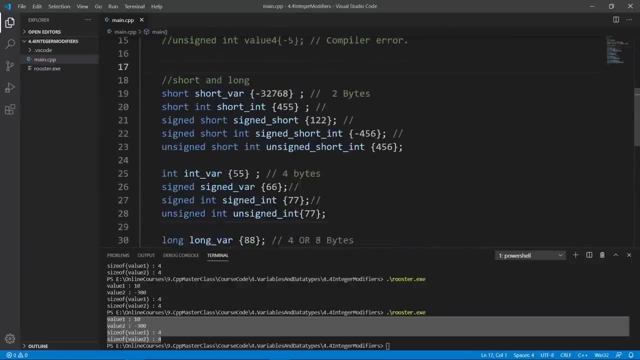 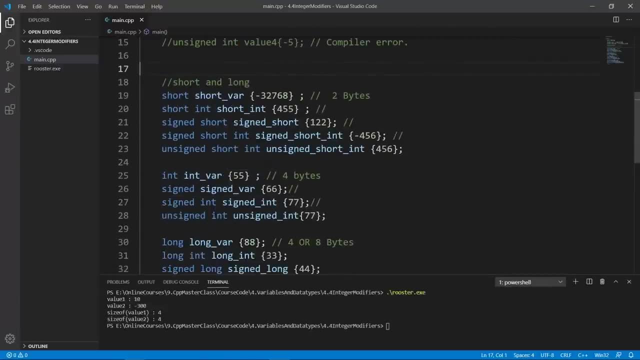 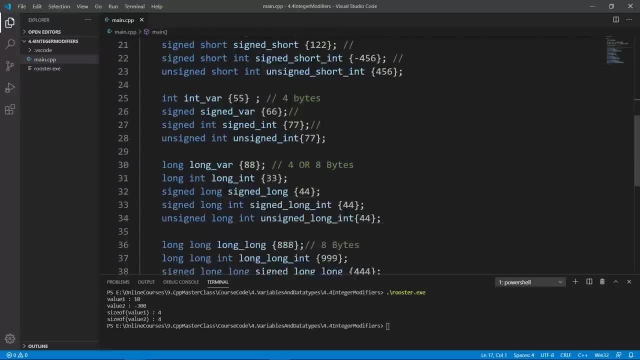 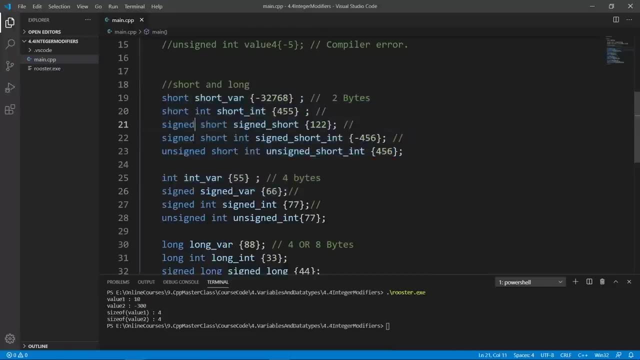 open the link, use the code, copy the code and paste it in here and really play with it, because the point is really not to type all this. the point is to understand what these modifiers do to your variables. what we are going to do, we're going to try to print them out and print the size they 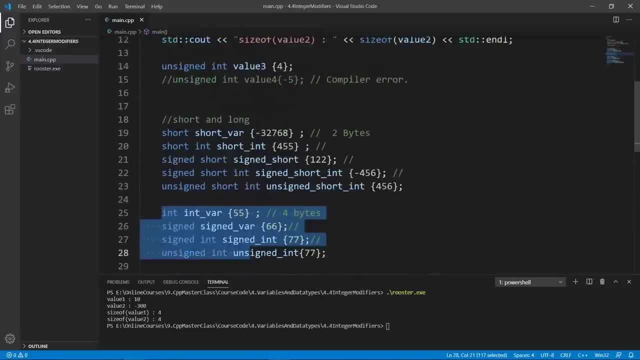 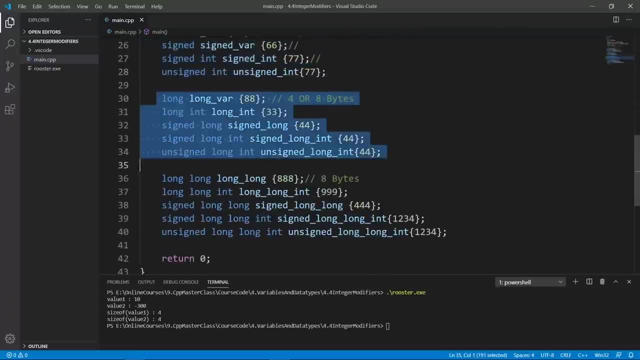 actually have in memory. we're going to do this in four groups. we're going to do one for short and long, we're going to do one for and here we're going to do one for long and we're going to do one for long, long. these are things. 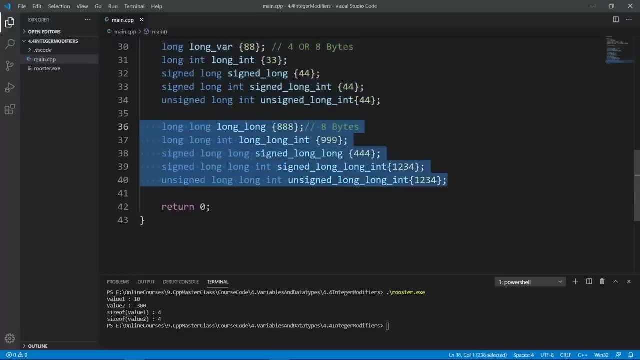 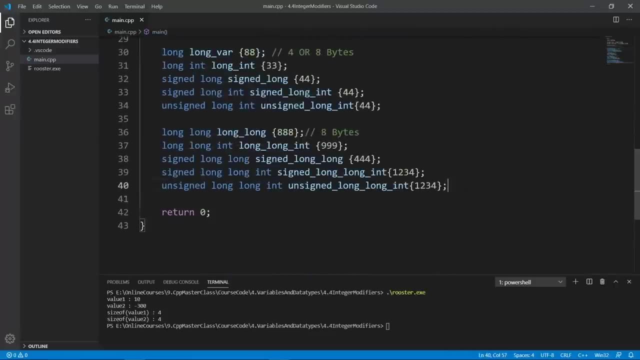 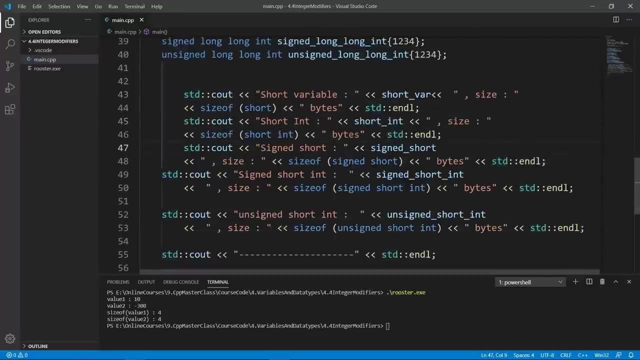 you can do, and we're going to see how much memory is actually being used by all these variables. we are going to start with the first group here, so we're going to go down and print the sizes out, and this may be really hard to wrap your brain around, but they are plain old std. 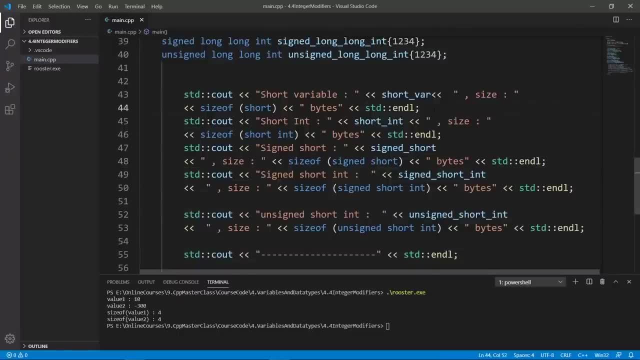 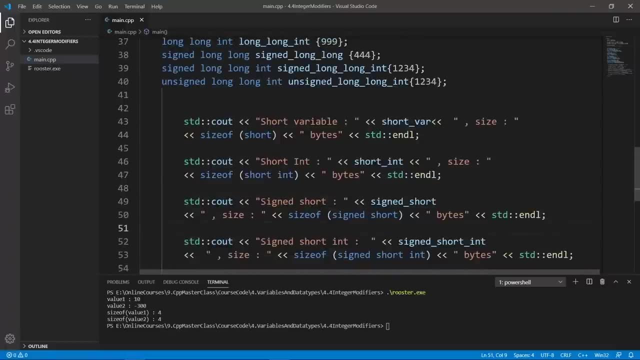 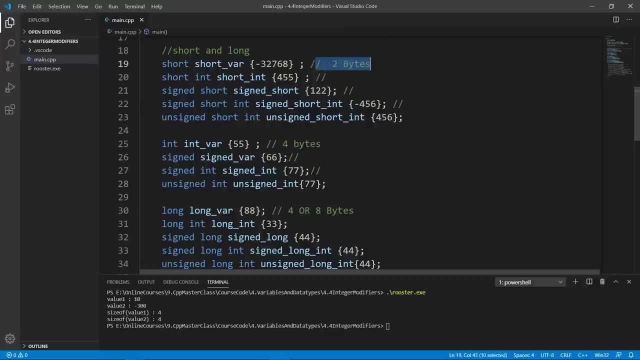 c out statements that we have been doing all along. i am going to split this on different lines so that you can really see this. so we have an output statement for a short var, which is what we have here. so we expect this to take two bytes and all these things are probably. 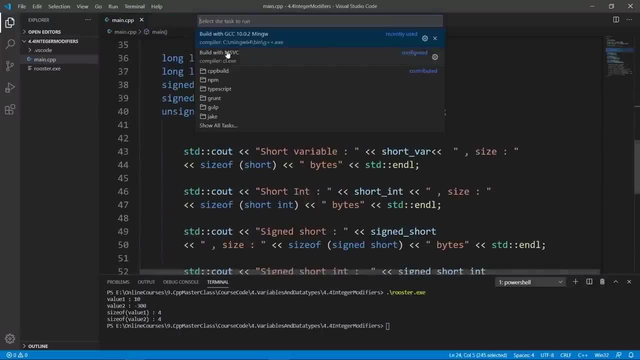 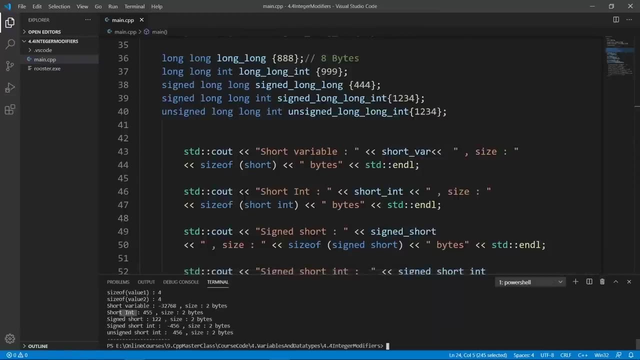 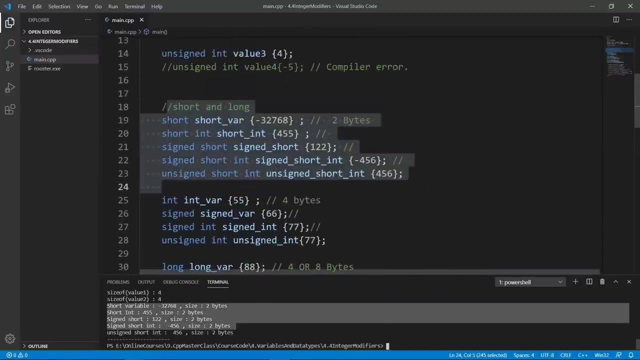 going to take two bytes. let's try and build the program with gcc. the world is going to be successful. we are going to run rooster and you're going to see that short end is two bytes, signed short is two bytes and everything is basically two bytes in this group here. and we did guess right. the next thing we want to try out is this: 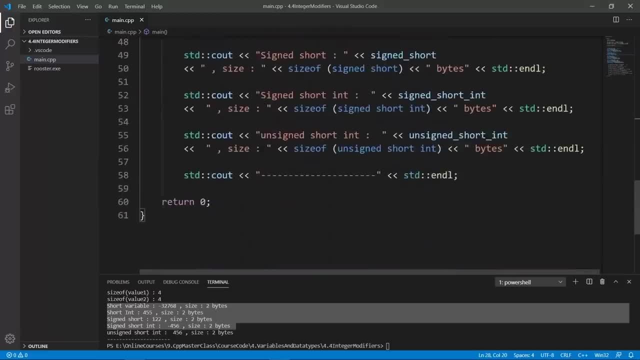 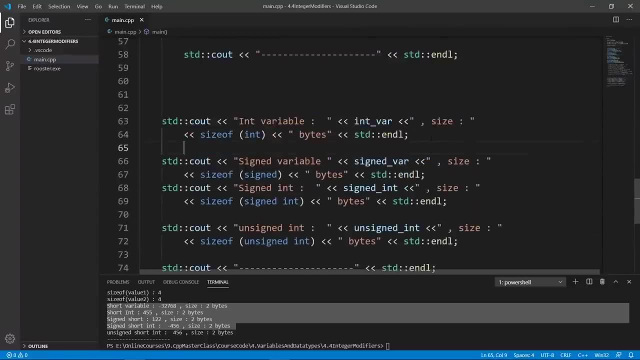 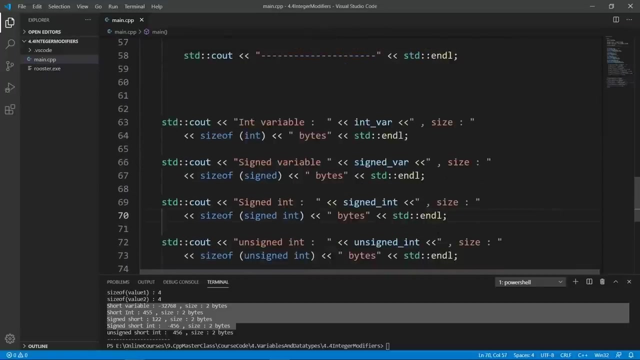 group of ends. so we are going to go down and give ourselves some breathing room and we're going to paste this in and we're going to separate these again so that we can see what is really happening here. and i think this is really enough. so we're going to see the sizes for the thanks we have. 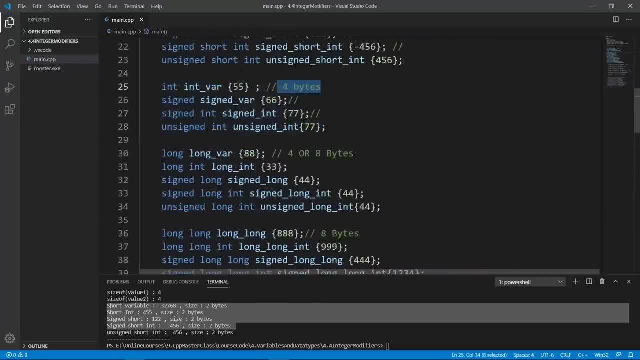 in this group here and we expect this to take four bytes. so we're going to go down and we're going to. so let's try and run the world task to world. with gcc. the world is going to be good. we can run the program like we usually do and you're going to see that ant variable is four. 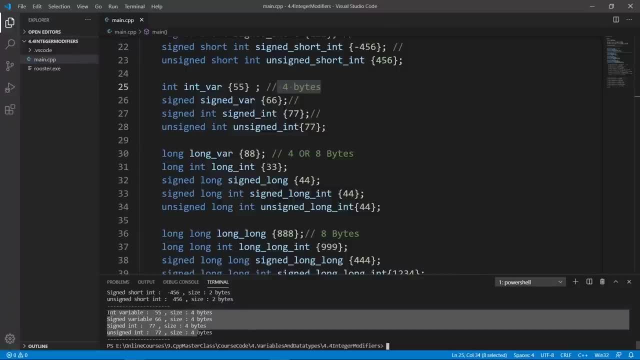 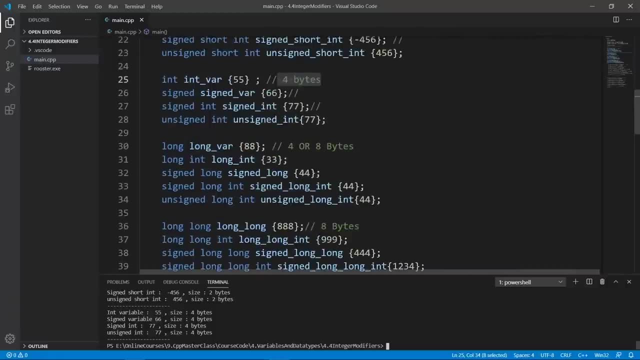 bytes and everything, and that group is four bytes and this tells you that, regardless of the signed and unsigned modifiers you put here, it's going to really use the size of it here. okay, it's going to four bytes in the memory. let's try this group here. we are going to go down and put in the code. 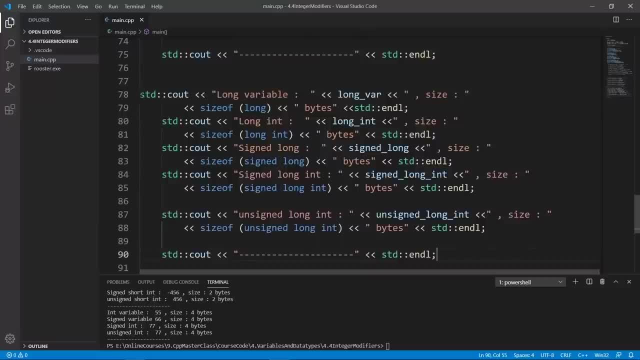 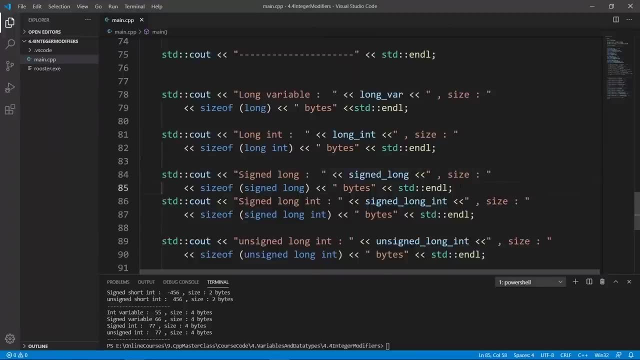 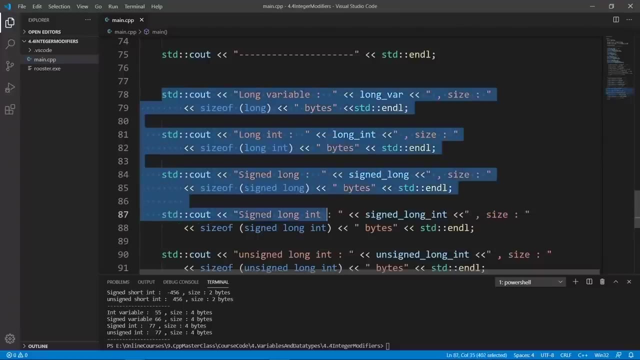 to print the sizes for them, and this is what we should use. let's split this on different lines so that it is easier on the eyes. and again, if you don't really want to type this, you can get the code from the linked resource section. you're going to find the code here and 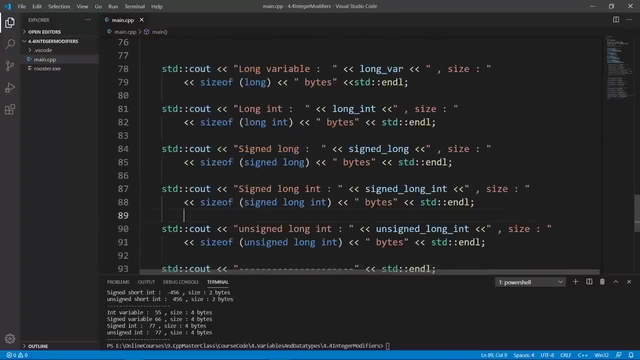 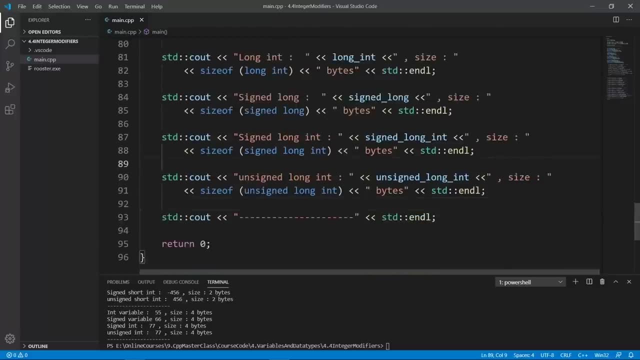 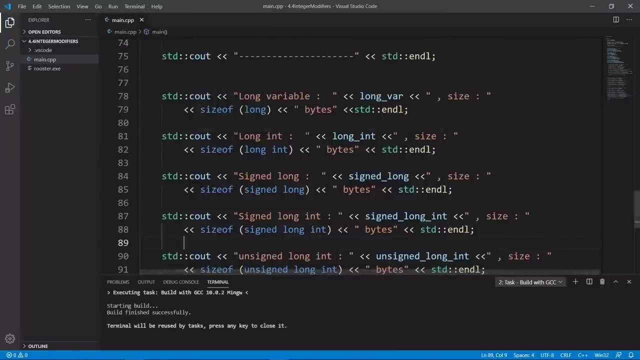 you can copy and paste and really play with us, but it is helpful to really type these things out and really bring these things in muscle memory because it's going to help. okay, so we have this n. we're going to try and run the build task with gcc. the build is good, we're going to go in here. 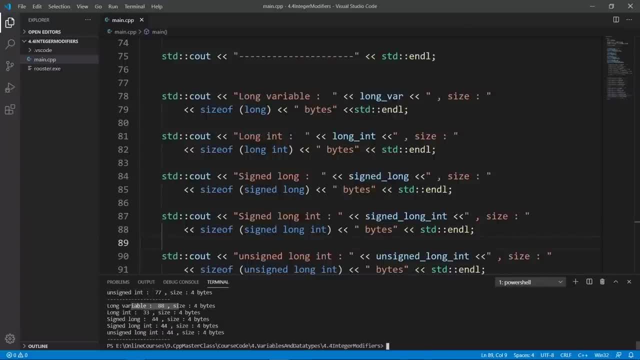 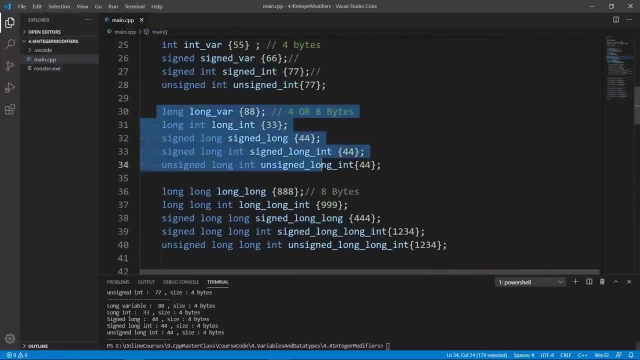 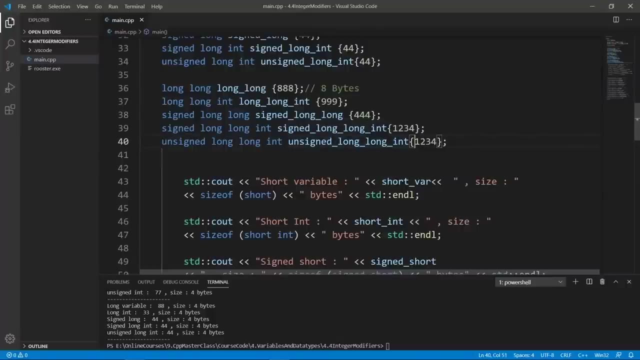 and run rooster and it is going to say long variable is four bytes and everything in this group is basically going to be four bytes in here. the last one is this long, long thing. it is going to really give you a huge range for your values you can store in the variable, but don't really 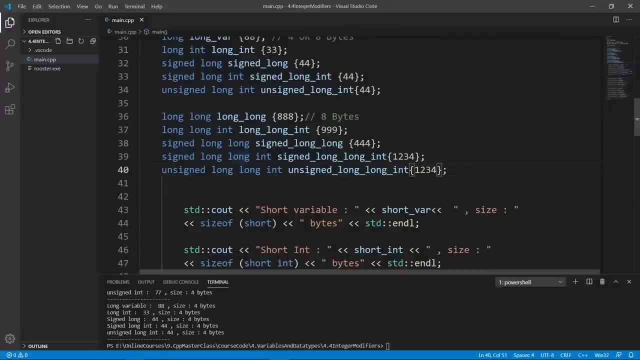 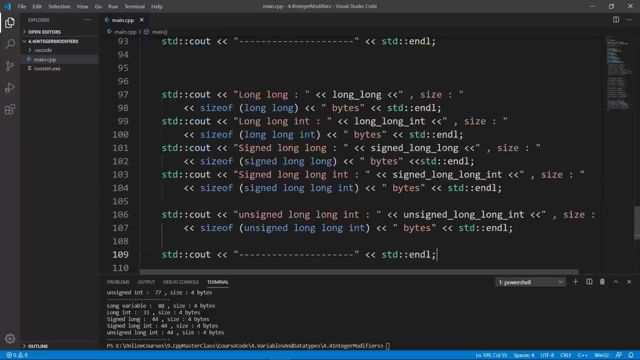 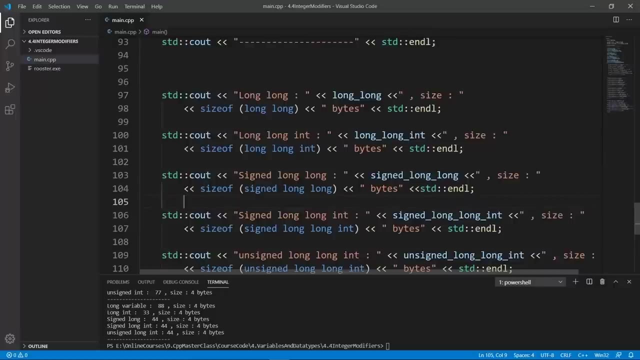 trust my world. let's try this out so that you can see for yourself. we are going to go down and really put this n, so we're going to give ourselves some breathing room and paste the code in. so i am going to bring this to the next line, and what we are really doing is printing the sizes for the variables. 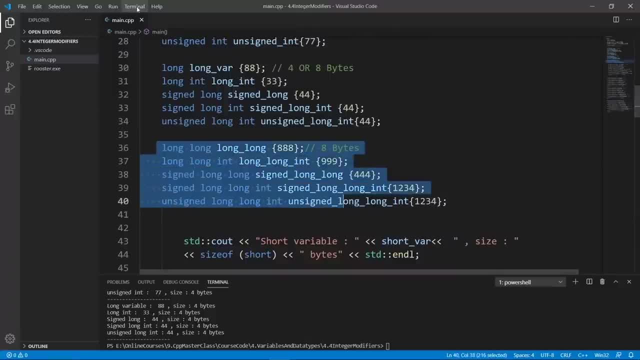 that we have in this group here. let's build and see if this passes the world. the world is going to be good. now we can run rooster and we're going to see that long long is eight bytes. eight bytes gives us a really huge range of values. okay, this is really all we set out to do in this lecture. 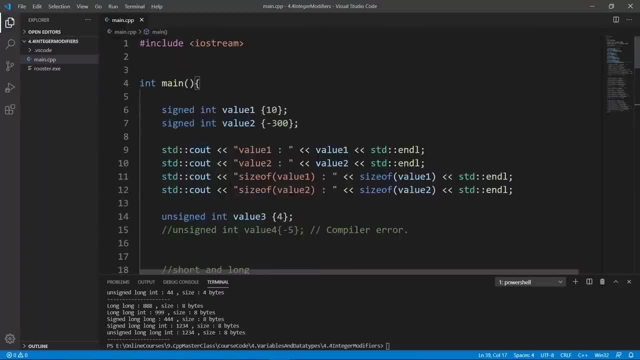 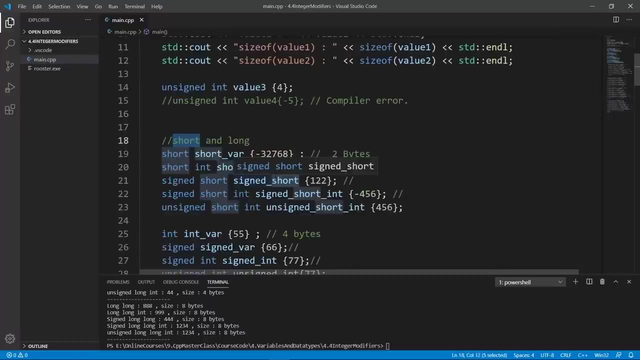 to learn about these integer modifiers. they modify the way your integer variables behave. for example, we can specify that we only want positive numbers, that we want to both store positive and negative numbers. for that you're going to use the signed or unsigned modifiers. you can also shorten or lengthen the range of values you can store in. 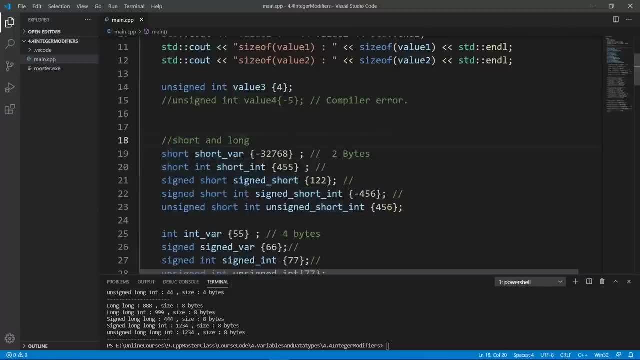 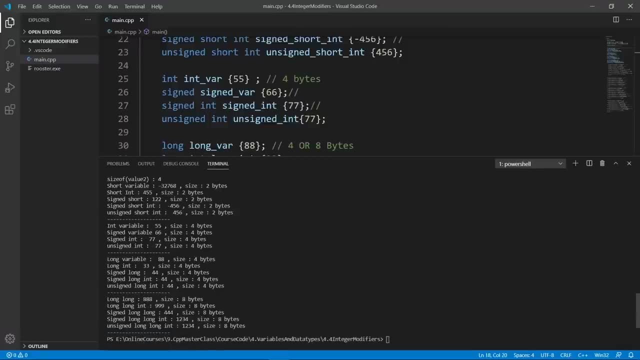 your variable by using the modifiers short and long and from the output of a program. here you can really see all these effects here. this is really all we set out to do in this lecture. i hope you found it interesting. we are going to stop here in this lecture. in the next one we're going to 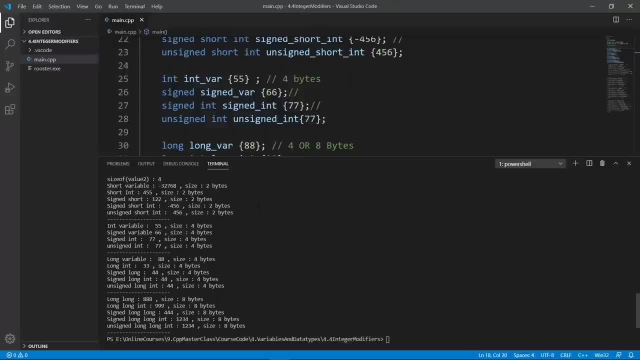 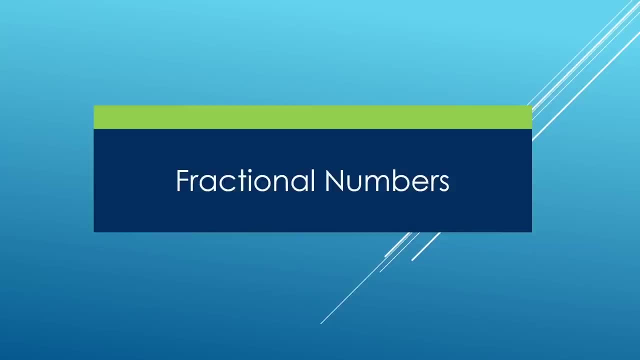 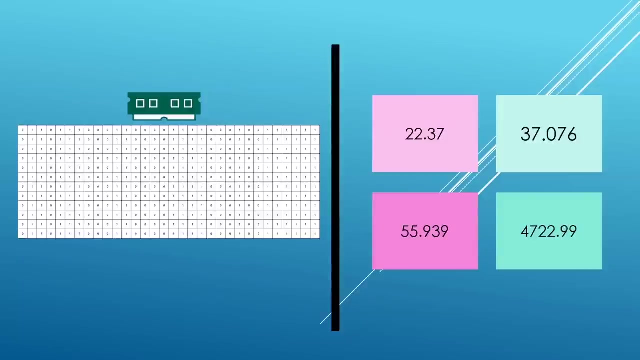 start and learn about fractional numbers. go ahead and finish up here and meet me there. in this lecture, we're going to learn about fractional numbers and as we work with these numbers, i want you to keep in mind that any piece of data you work with in your c++ program is ultimately going. 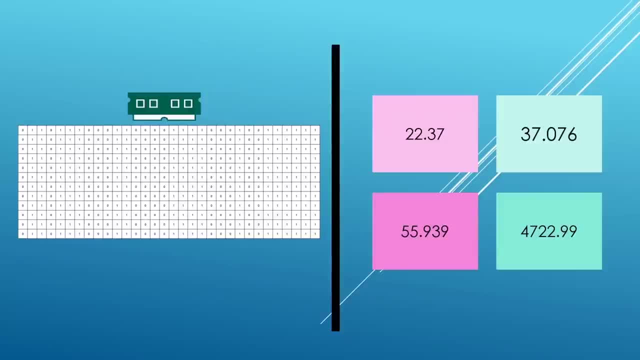 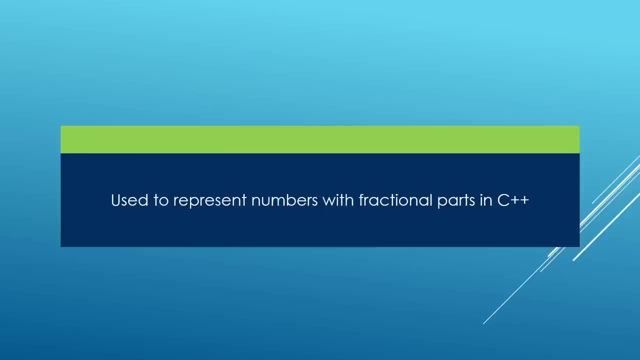 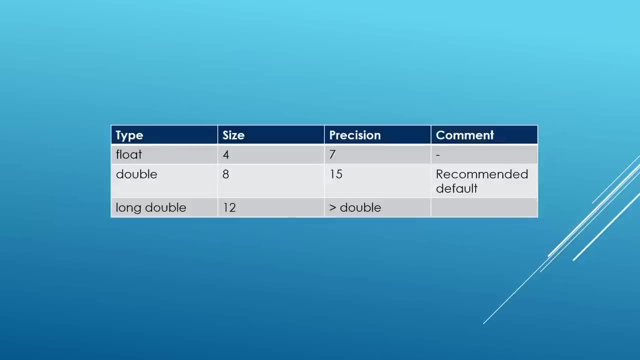 to be stored in the form of ones and zeros in memory. fractional number are also called floating types. in technical terms, they are used to represent numbers with fractional parts in c plus plus and many other languages, and we have three types that we can use. in c plus plus we have float double and long double, and the main difference is in the size. 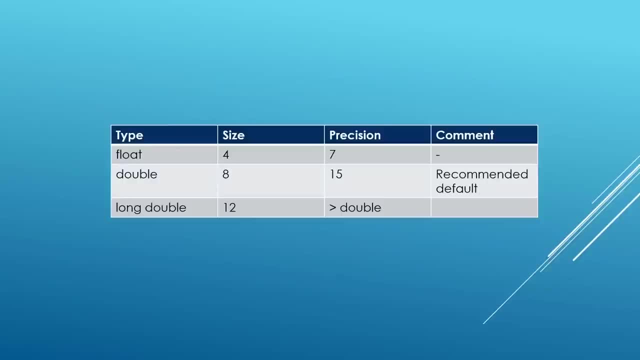 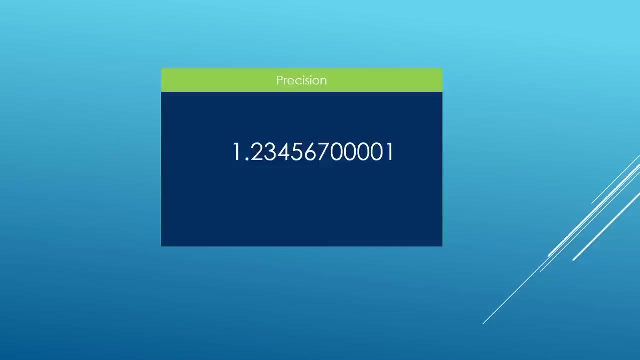 they occupy in memory. a float takes four bytes, a double takes eight bytes and a long double takes 12 bytes typically. so as the size goes up, you can also notice that the precision goes up. so what is the precision? the precision is basically the number of bits you can represent with that type, starting from the. 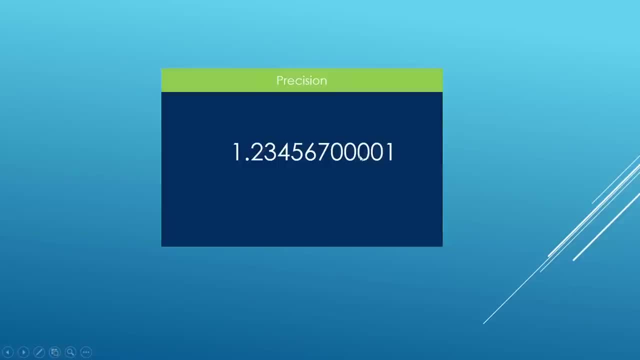 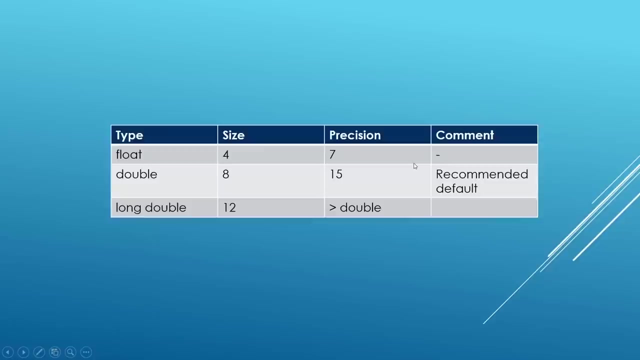 number in front of the decimal point. so if we look at this number here, we can try and figure out its precision. so we're going to count one, two, three, four, five, six, seven, eight, nine, ten, eleven, twelve. the precision here is 12.. if we go back to our table, we're really not able to represent a number. 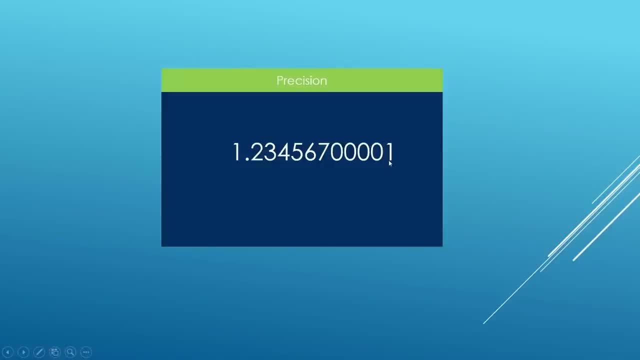 like this with a. the smallest thing we can use to represent this number well is a double, because the precision is 15 and it is more than what we need for this number, which is 12.. one thing you should remember is that the number in front of the decimal point is also counted in when you are trying to figure out the 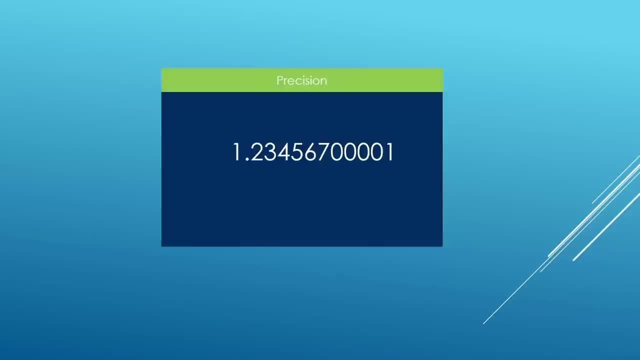 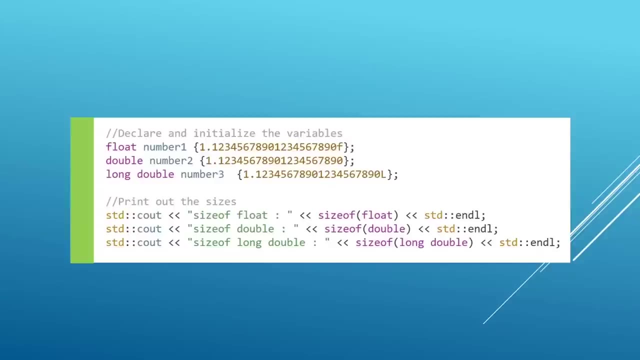 precision for your floating point numbers in c plus plus. so here we have an example of how we can declare and initialize floating point numbers numbers in our C++ program. number one is a really huge number, so you can guess that this is more than we can handle with the float. we're going to see how this is handled by our compiler, a double. 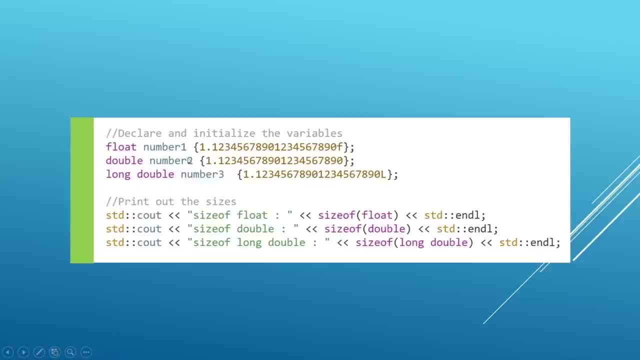 has a precision of 15, so we should expect to store more numbers than we did in a float. a long double should be able to handle this without a problem because if we go back to our table here, our long double here should be able to handle this better than double. but it is possible that it is the same. 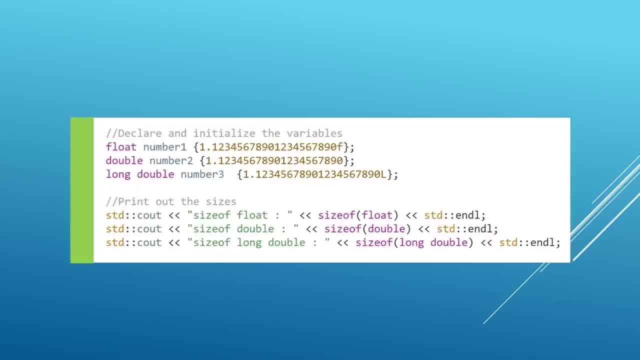 thing as double, depending on the compiler implementation. and if we try to print out the sizes here, we're going to see what the compiler gives us. we're going to do this when we try this in visual studio code. okay, and here we are trying to print out the precision of these. 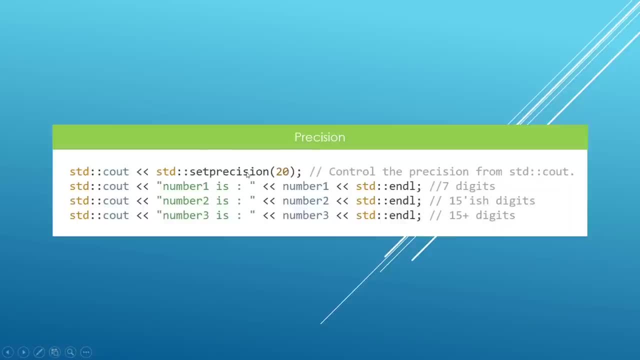 numbers. we can use a special setting on our stream to control it. the maximum precision that we can see here. you see that we are trying to show the precision for each number. there is a special setting we can put on stdc out to make it control the precision to a. 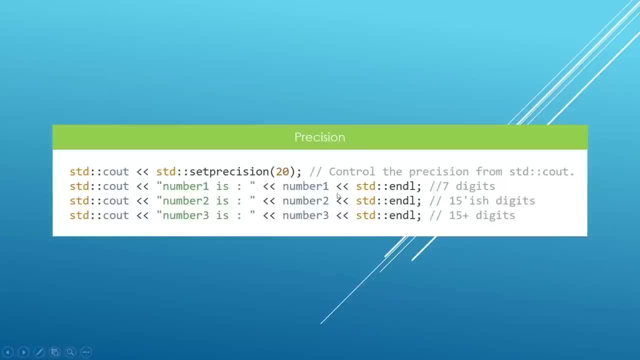 given number. here we are using 20 and we're going to see that for number one this is going to be seven digits. for number two it should be 15 digits or something close to that. the specifics are really dependent on the compiler implementation and for long double it should at least be the same. 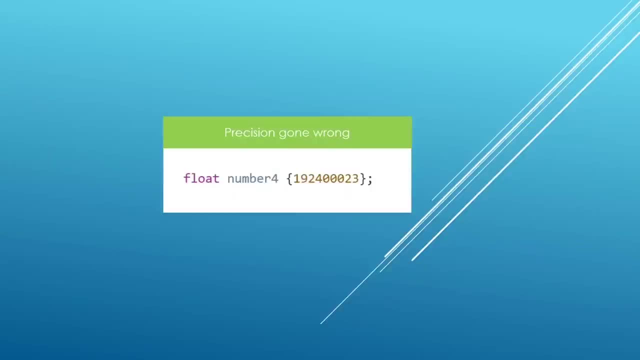 as double or even more in some cases. okay, here we want to see that we can also have narrowing errors if we try to store something bad in a float and a float can't really handle it. here we have a number with a lot of digits- one, two, three, four, five, six, seven, eight, nine- and we know that the float can. 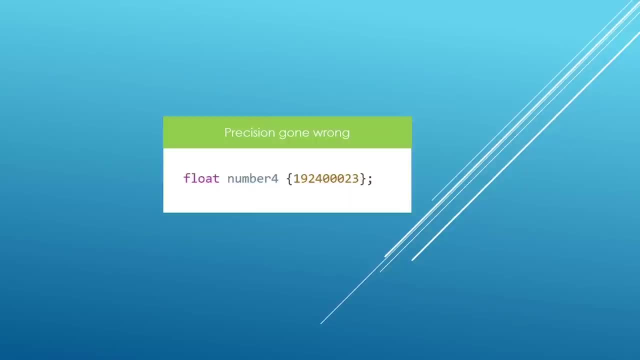 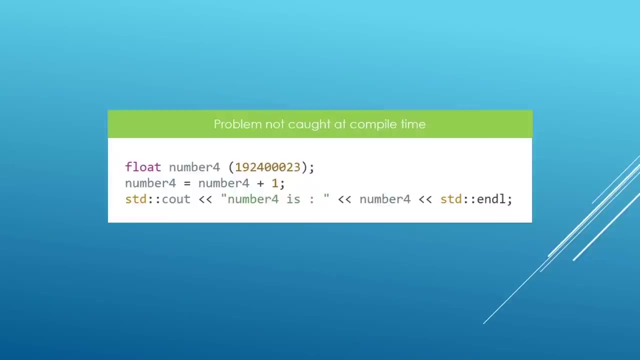 only handle seven digits. so this is probably going to give us a compiler error, as we've seen for braced initialization. if we use functional initialization, this problem is not going to be code at compile time, so we're going to end up with a chunked piece of data, and we're going to see this when we play with this. 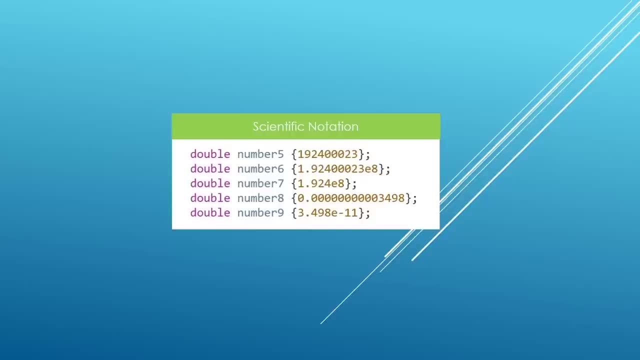 with visual studio code, and another format we can use with floating points is that we can use scientific notation and it is basically a way we can use a power of 10 multiplier to multiply with our floating point number. so for example, here number five is going to be this number one, nine, two, four, zero, zero, zero, twenty three we can use: 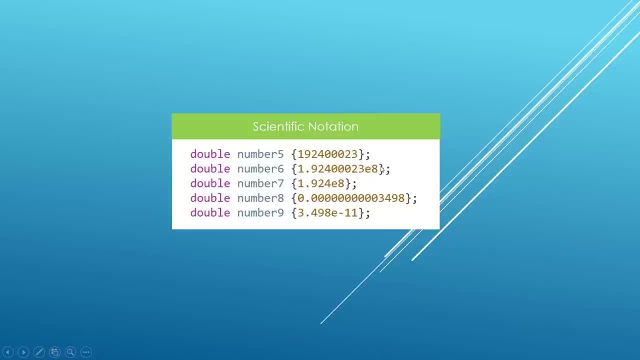 a floating point, scientific notation to represent this. so what we're going to do, we're going to say 1.9 and we're going to multiply this with 10 to the power of 8. this is what this means. this 8 here is going to be 10 to the power of 9. so we're going to multiply this with 10 to the power of 8, and 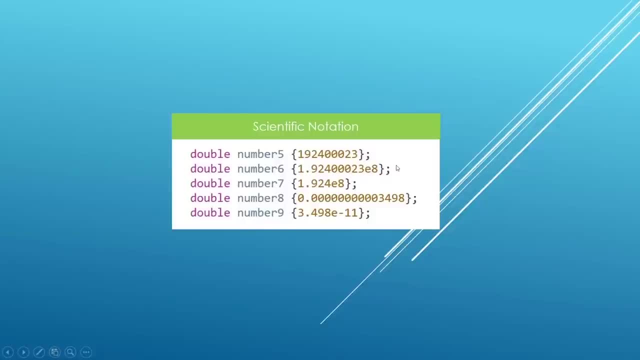 if we multiply with that, that basically means moving the decimal point 8 digits to the right, so we can go one, two, three, four, five, six, seven, eight, and it is going to end at these three here and it is going to be basically the same number. number seven is also another one and if we do this, we're 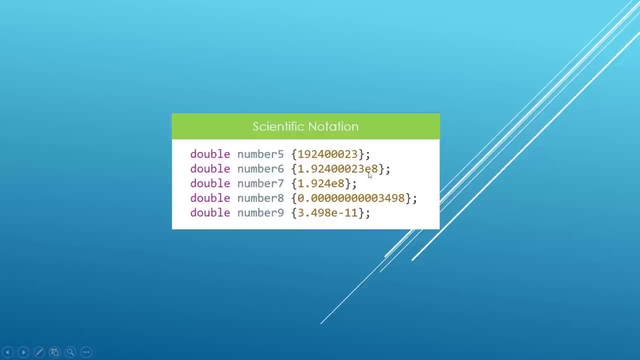 going to pad with zeros after these four and we're going to end up at this same location, but it is going to be a zero. we're going to see about that in a minute. and number eight is another floating point number and we can use scientific notation to represent it, just like you see with 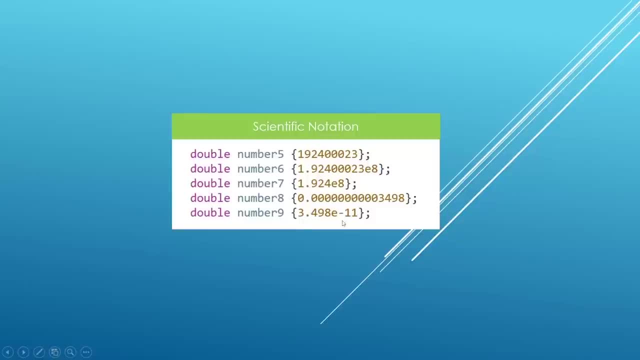 number nine. we're basically going to have the same thing when we have a minus in here. it means we're going to multiply with 10 to the power of minus 11, and this is going to give us a number below one- think 0.007 or something like that. so we're going to go 11 digits after the zero here. 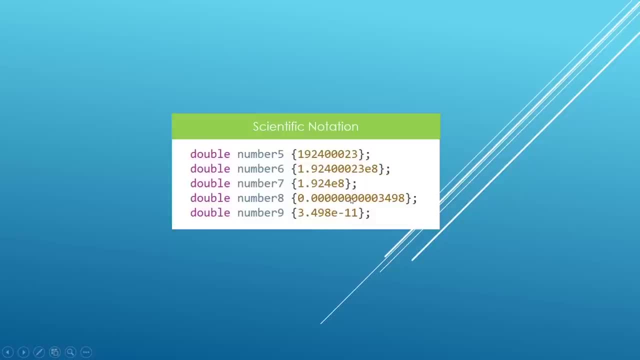 and if we count 1, 2, 3, 4, 5, 6, 7, 8, 9, 10, 11, and the decimal point is going to go after three and we're going to basically end up with the same thing here. we're going to play with this in a 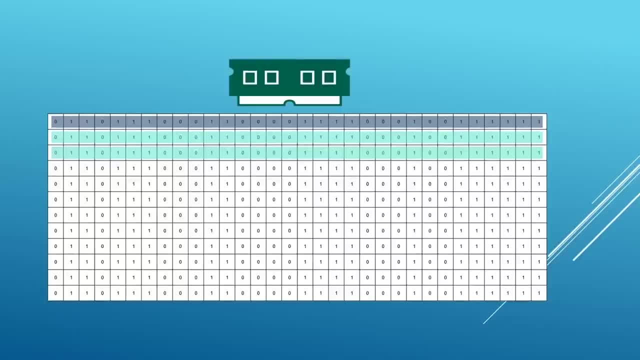 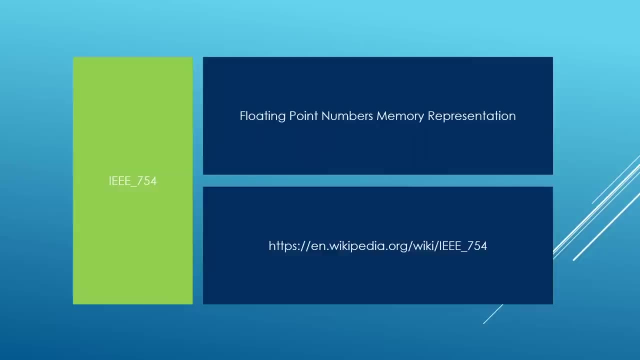 minute and you're going to see that all this makes sense. and don't forget that any piece of data we store in a computer is going to be ultimately represented by ones and zeros in memory, and for floating points we don't use the number systems like we've done for integers. there is a special system that is used to do that. 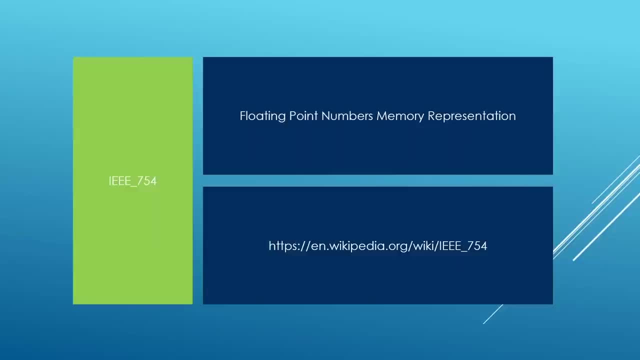 but it is a little bit complicated to cover in a course like this. i am just going to point you to it. if you are interested, and when you are done with this course, you can come up and read on this. the main point is that any piece of data that you represent in your c++ program 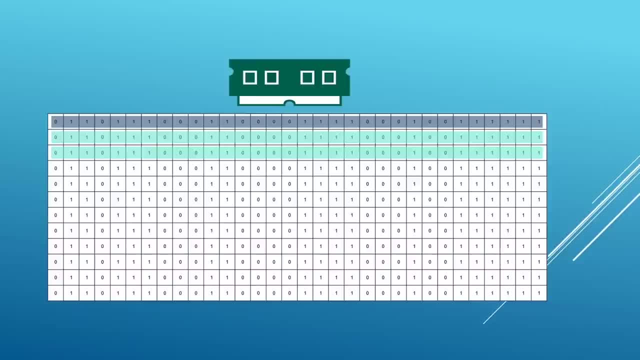 is going to be represented by ones and zeros in memory, and for floating points we don't use the. the main point is that any piece of data that you represent in your c++ program is going to be represented in terms of ones and zeros in the memory of your computer. okay, there are a few. 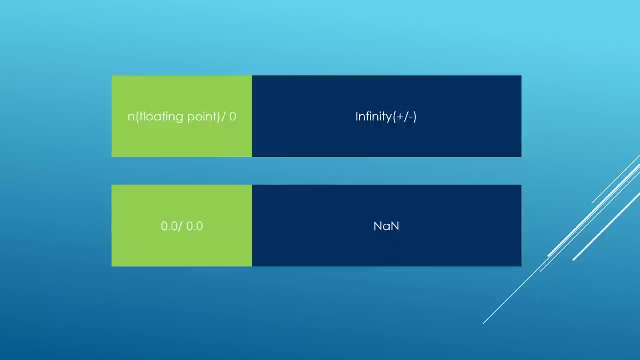 things you can do with floating points that you can't really do with integers. for example, you can divide with zero. if you take a floating point number and divide that with zero, you're going to get what we call infinity. if the number is positive, you're going to get positive infinity. 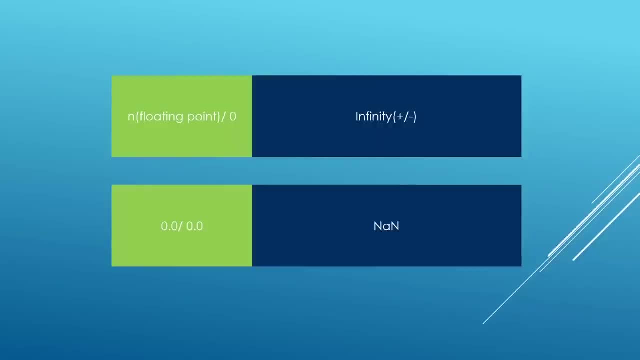 if the number is negative, you're going to get negative infinity, and you can take two floating point numbers that are zeros and divide them, and what you're going to get really is not a number. it's something called nan, which stands for not a number, and, uh, your program is going to not crash. 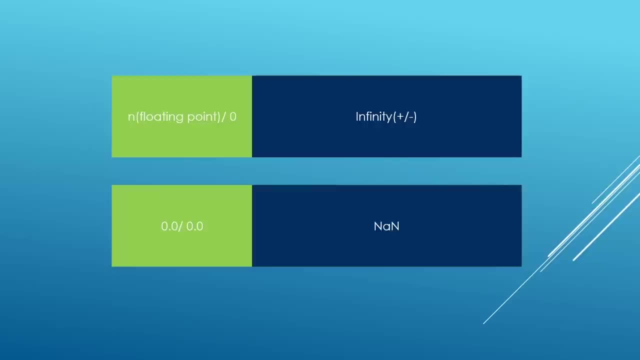 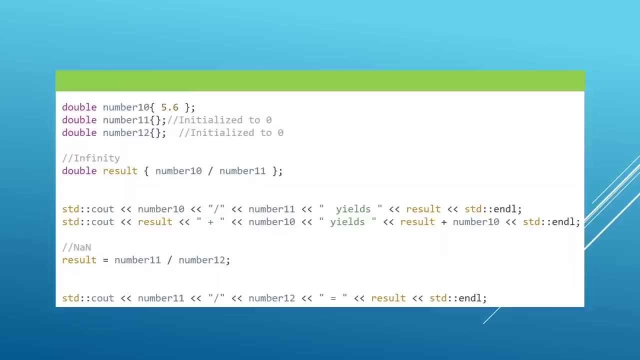 but there are a few things you can't do with these things. for example, you can't add them up. you shouldn't really do this. it's probably going to end up bad for your program. here we have a few examples. we have three numbers declared. they are doubles. they must be occupying eight bytes in. 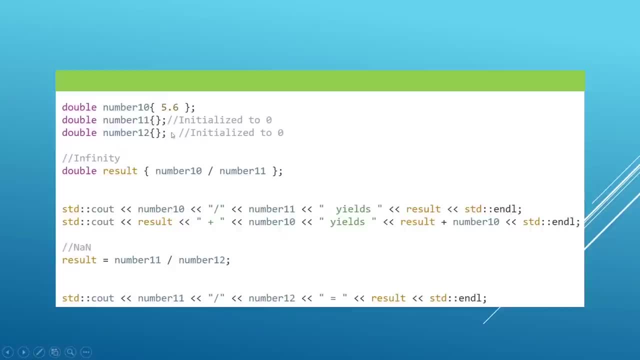 memory. now we have a few examples. we have three numbers declared. they are doubles. they must be occupying eight bytes in memory. number 10 is initialized to 5.6. 11 is initialized to zero because we are using the braced initialization and we have nothing in here and uh. infinity here is the result of dividing. 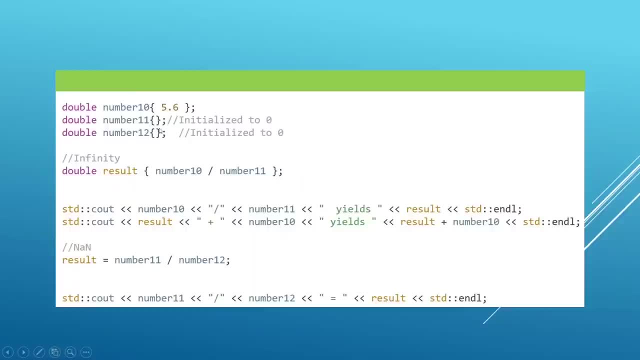 a number by zero. so it's going to be positive infinity because number 10 is a positive number. if you go down. we're going to print number 10 divided by number 11 and we're going to say yields. we're going to put the reserve out. we're going to see that down here. 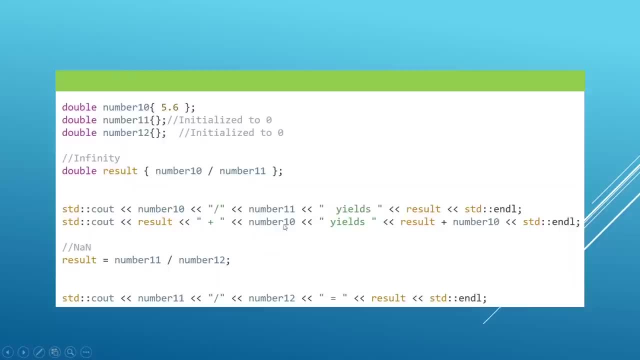 on the second line. you see that we are trying to add something to infinity and this is also going to yield infinity, because think of infinity as something super big and if you add something small to something big, it's still going to be something big down here. you see that reserved. 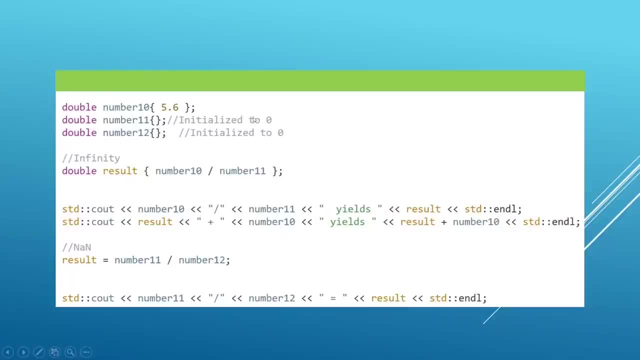 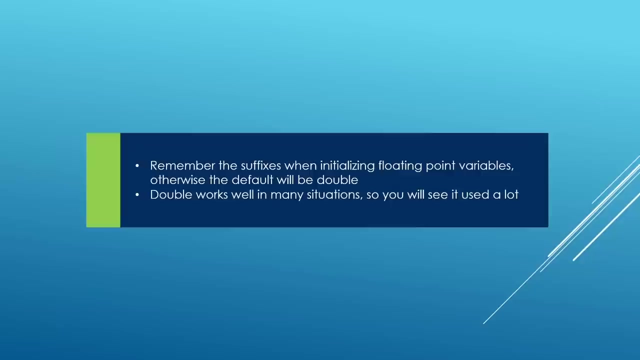 equals number 11 divided by number 12, and these two are zeros, so we're going to end up with none, and that's what we're going to print in this statement here, down to the bottom. okay, you should put in the suffixes when you are initializing your floating point numbers, otherwise the default is. 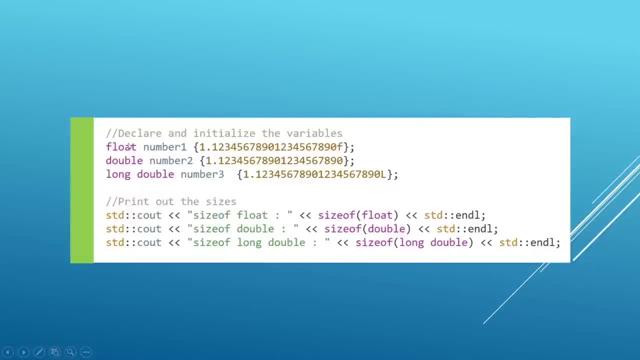 going to be double. this is what we mean by this. you see, this floating number, we have a suffix, that is f, to mean that it is a floating number. if you don't put that in, this is going to be interpreted as double and the compiler is going to try and turn that into a float by chopping off. 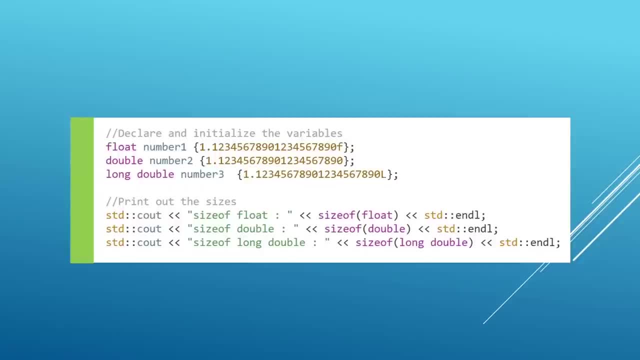 things that can't really fit in a float. so to really make it clear that you are storing in a floating number, let's put this f suffix here. for double you don't need to put anything because it is the default assumed by the compiler. but for a long double you have to suffix this with l, just like this. so 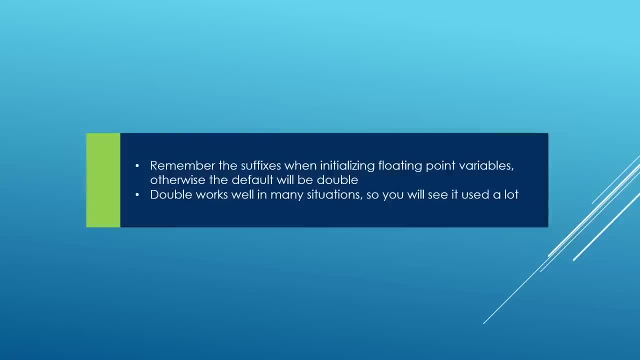 that's what we really mean here. we have seen that the precision for float isn't really enough for many of the computations we might want to do in our c plus applications. okay, we have talked a lot about floating point numbers. let's head to visual studio code and 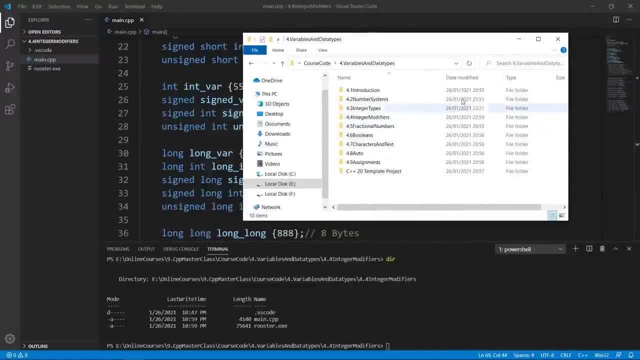 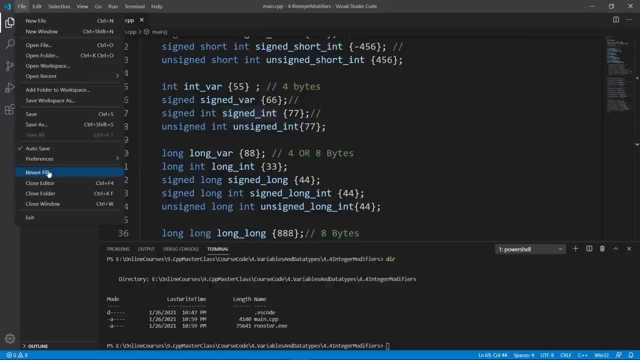 actually play with them. okay, here we are in our folder that is going to contain our project. the project is going to be called fractional numbers. so we're going to copy our files, go up a little bit and put those in, and we're going to go up again and open this in visual studio code. we're going 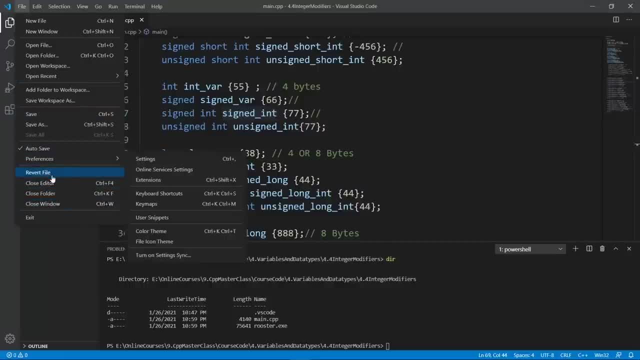 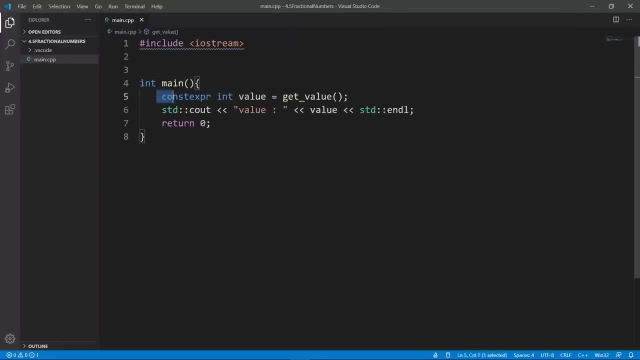 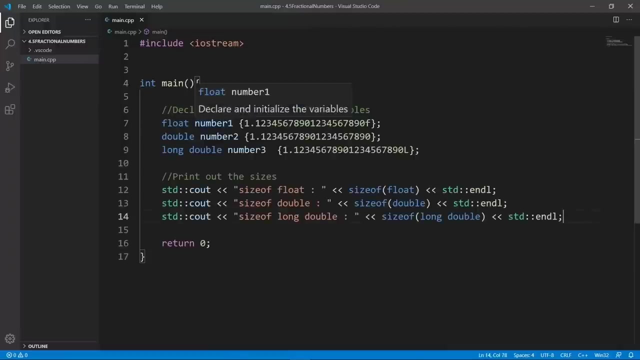 to close whatever it is we have opened. now we're going to close folder and we're going to open our project in visual studio code and we're going to do the usual and remove things we don't need in. the first thing we want to do is to store a few floats in our program. we're going to declare and: 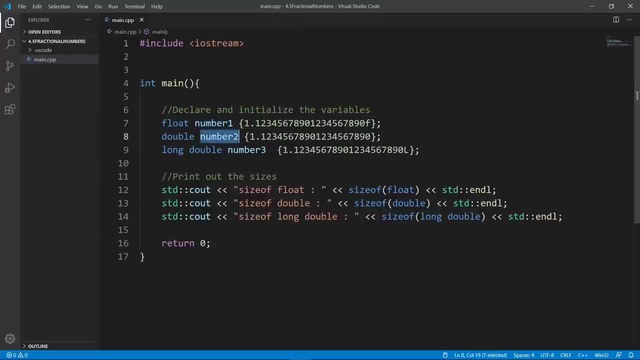 initialize a few floating point numbers. we have number one, number two and number three and we want to make it clear that the sizes are what we expect. we are going to open a terminal window here and we're going to build with gcc. run the task to build with gcc. the build is going to be successful. we're. 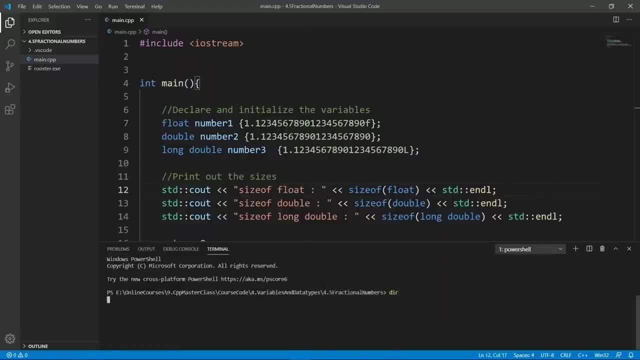 going to come to our terminal, click a little bit and we're going to type there. we're going to see that the size of float is four, size of double is eight and size of long double is 16.. this is what we expected. another thing we can do is try and play with the precision of these numbers and see: 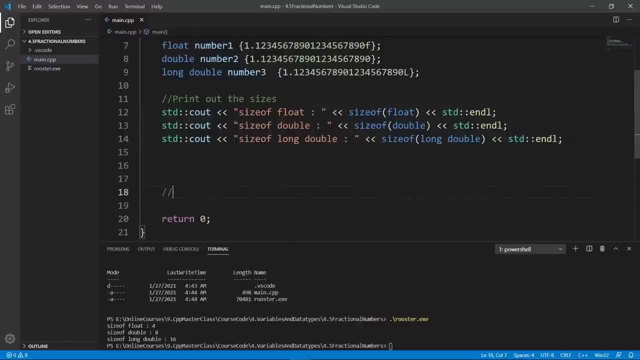 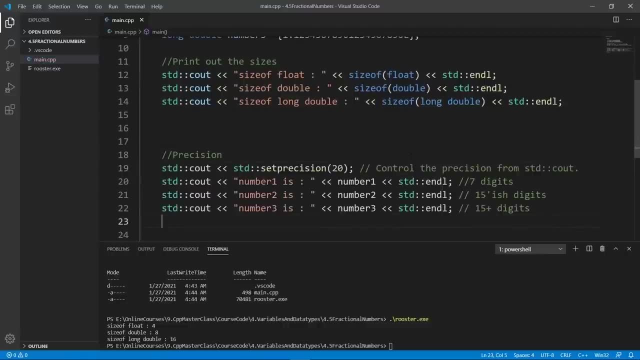 what we can really go away with. okay, so we're going to actually put in a piece of code to play with this. we're going to add a setting to our sddc out stream so that we can control the precision, and we're going to add a new setting to our sddc out stream so that we can control the precision. 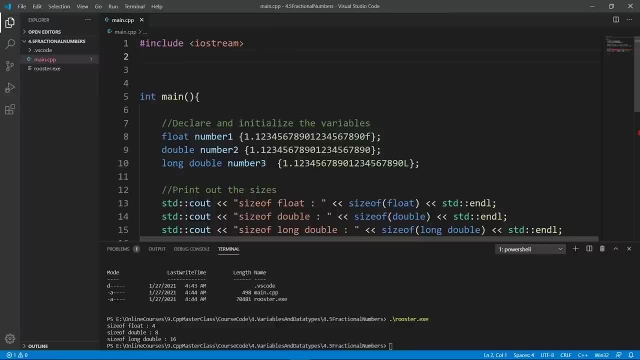 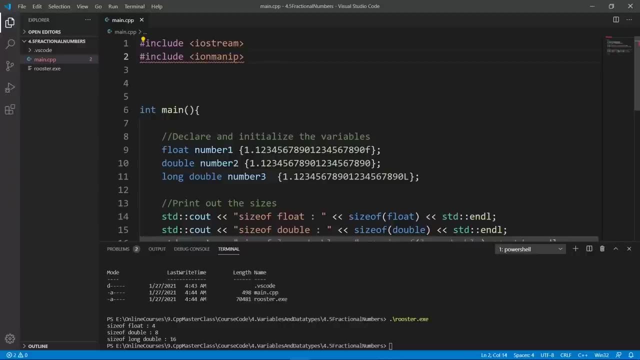 but for this to work we need to bring in a library that is called i o money. so we're going to include that i o money. and how do i know this? i usually consult the c plus plus standard library documentation and you are not at a point where you can really understand it right now. so we're going. 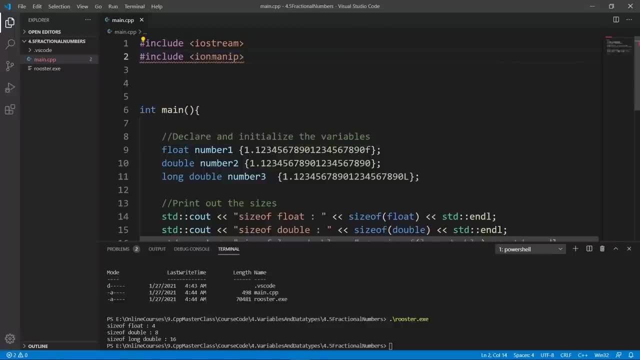 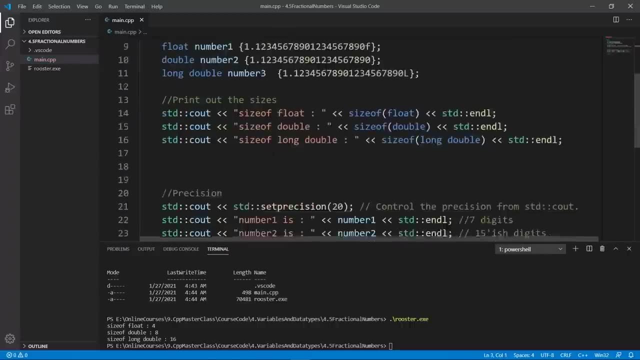 to be putting in these things here and explaining them as we go. and i made the type here. it is i o manip, and you see that now this is recognized, or program should compile. so we're going to try and weld it so that we can try this out. we're going. 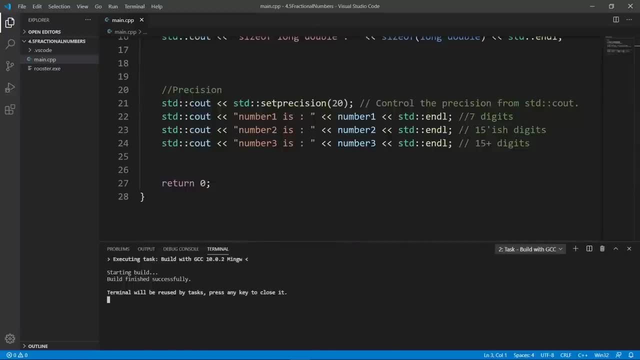 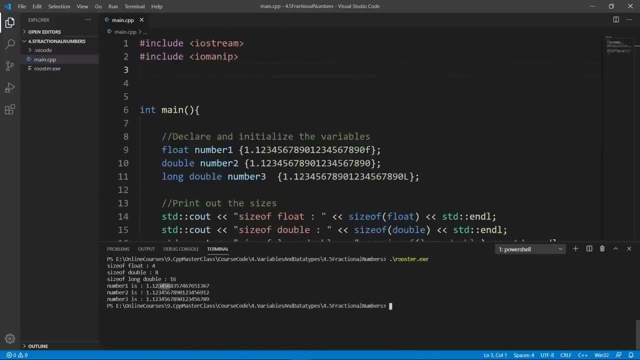 to weld with gcc. the build is going to go through, we can run our program. we're going to do there and clear and rooster to run. you see that things start to go off at sex and if we count what we have here, it is one, two, three, four, five, six, seven. we can only represent seven numbers accurately. 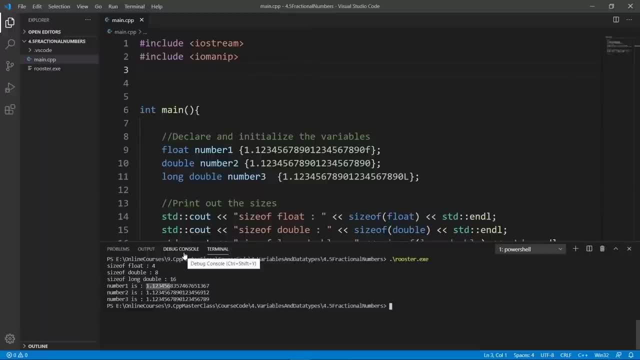 with a float and after that we're just going to have garbage because the computer can't really make sense of whatever we have after our seven digits that we can legally represent with the float. so the precision for our floating point number here is seven. i really hope. 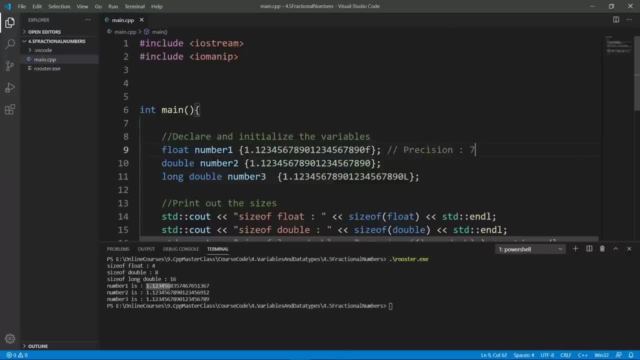 this makes sense. let's check out number two. we are using double, so precision should be around something like 15. so we are putting in a number one through nine and we are starting over zero. one, two, three, four, five, up to zero again. if we look at, 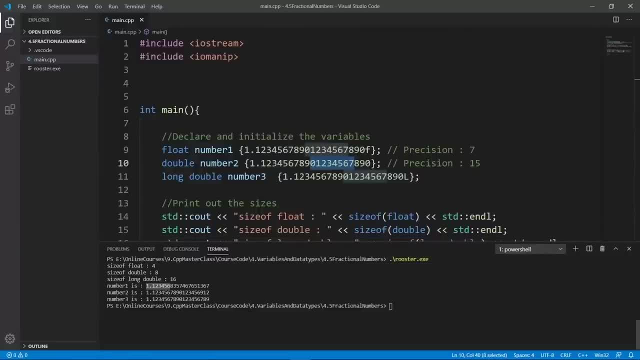 what we have in the output. here we have one, two, three, four, five, six, seven, eight, nine, zero. one, two, three, four, five, six, and here things start falling off after our six year, and if we count, we're going to have one, two, three, four, five, six, seven, eight, nine, ten, eleven, twelve, thirteen, fourteen, fifteen. 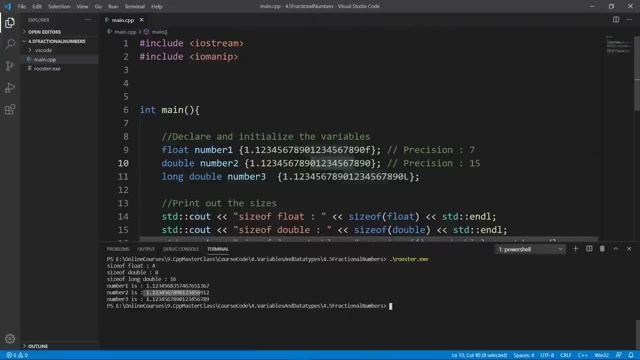 sixteen, seventeen digits. this is the precision. we are having this compiler here. it is around 16 and it also shows that the double is 17, so it is something around 15, and we should expect to have something more than that, or at least the same thing as double with. 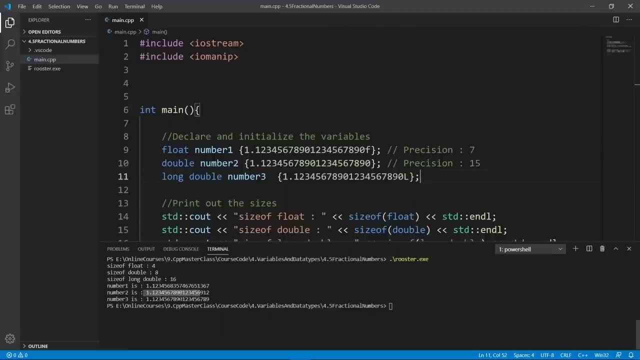 long double. so if we look at this, you see that it is one, two, three, four, five, six, seven, eight, nine, zero. one, two, three, four, five, six, seven, eight, nine. we are able to represent up to 20, and you can see that long double leaves up to even the precision of 20 that we have here. so this is something that we can. 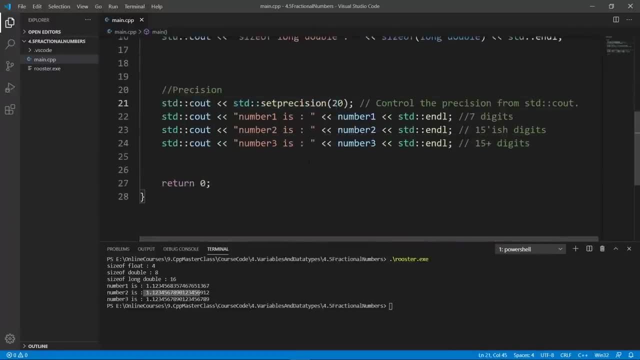 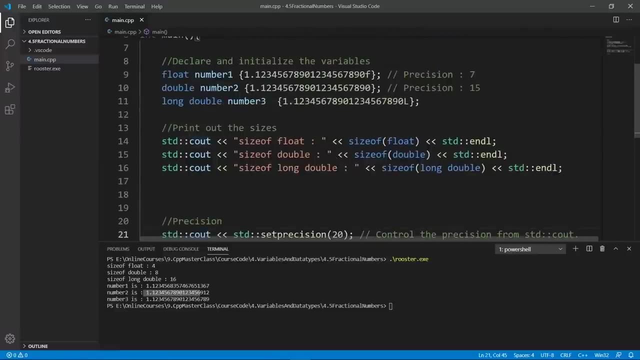 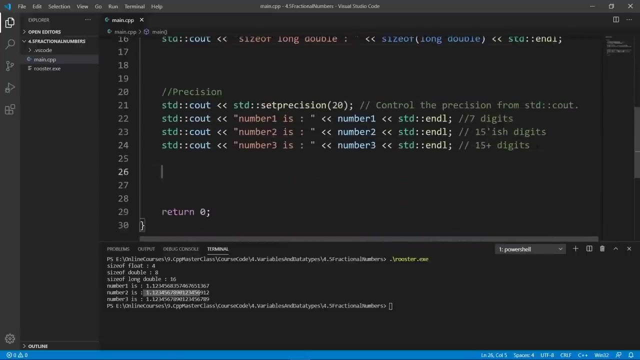 we have set with std set precision here. okay, i really hope now that you have an idea about these precisions we have with our floating point types in c plus plus programs. another thing i want you to see is what kind of narrowing errors we can get if we try to initialize with something that 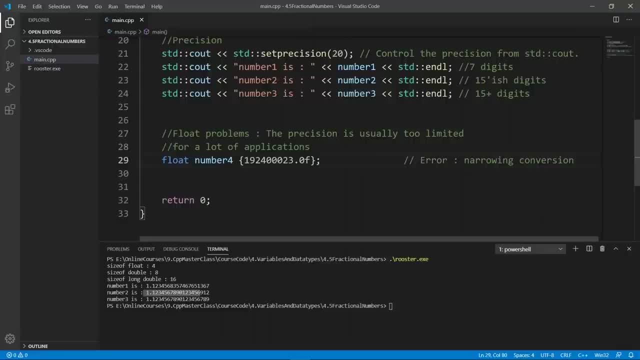 can't really be represented by a floating point number, and here we have a float. it is called number four and we are trying to put in something that is bigger than we can really fit in. it has more than seven digits, so one, two, three, four, five, six, seven, eight, nine. it is more than seven digits. 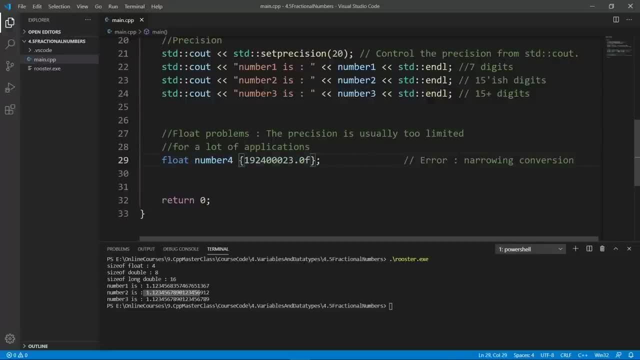 and we would expect to have a problem with us because we are using braced initialization. let's try and build this with gcc. we're going to do that and this is going to work successfully. so this is going to silently chop off our number if we try to print it out. 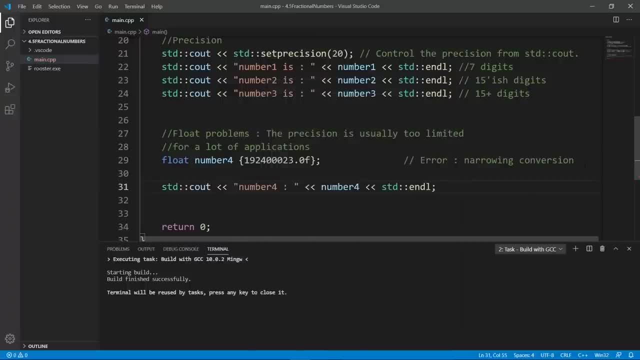 we're going to say stdc out number four and we're going to build again, run the test world so that our changes are taken into effect. i'm going to do there and do rooster and this is going to print our number. you're going to see that after the zeros we have junk. our number has been basically: 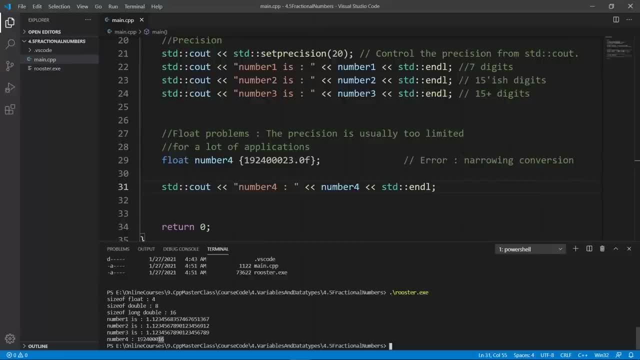 chopped off, and this is junk because we can't really represent this with the double. the 16 here has been chopped off because we can't basically represent this with the floating point number. if we change this to double, this is going to probably give us what we expect, so let's run again. world. 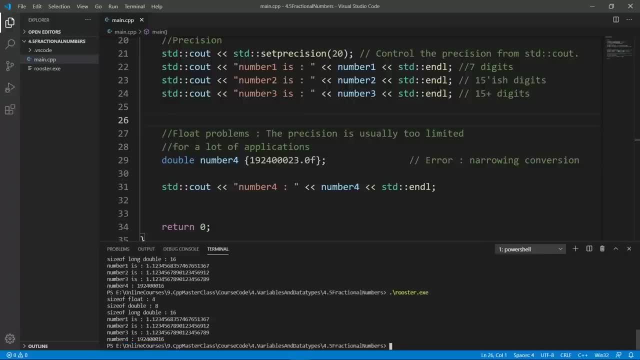 with gcc. the world is going to be good. if we run the program, it is going to show us the same thing. okay, this is a really good learning change. why are we having the same results as before, even if we changed the type to double? try to think about it. the reason is the suffix here is still saying: 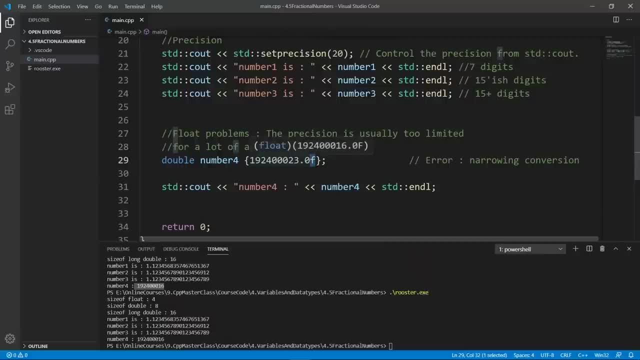 f and this is going to be stored as float in memory. so if we want this to really be treated like a double, we can take out the float here and if we build again and run the application now, you're going to see that we see the 23. this is basically. 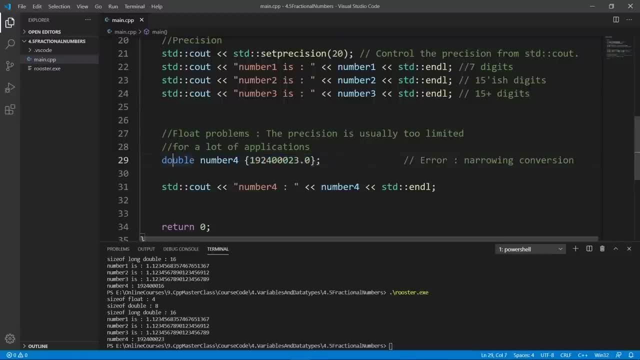 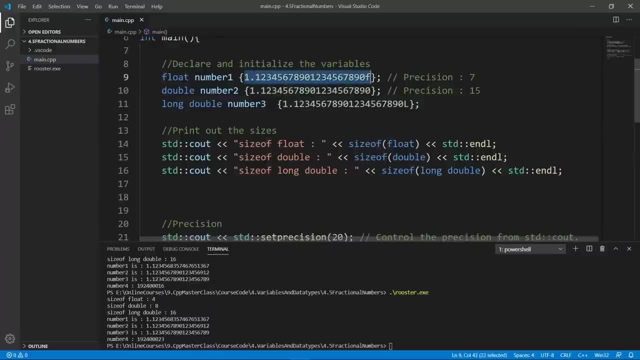 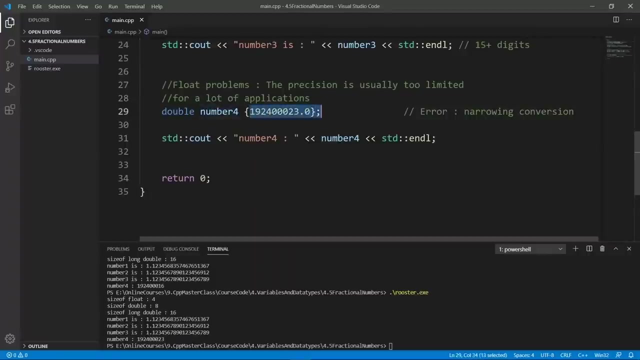 being correctly stored as a double. this is a really good thing you should keep in mind. if you don't put in your suffixes here, the number is going to be interpreted as double by now. i hope you see that if you really try to put more than your floating point can. 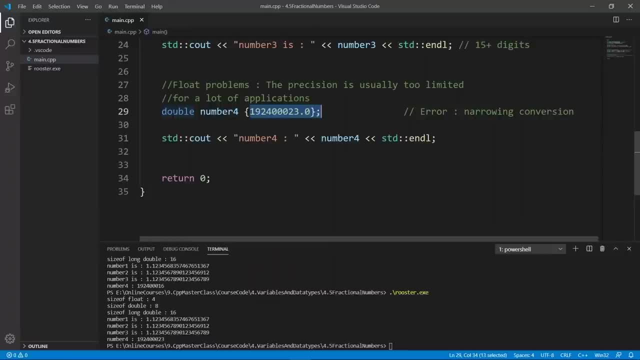 handle. the number is going to be chopped off and only the precision that it can handle is going to be stored in. i hope this makes sense and you see that the behavior for numbers is really different. we got the compiler error when we try to do narrowing conversion with integers. 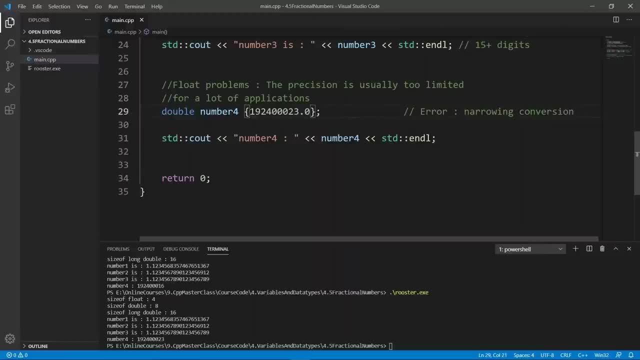 but now it is silently chopping off our number. if we try and use functional notation, i think we're going to get the same result and change this back to a float and use float here. and if we build again, let's go to terminal run task, use gcc. we're going to run this. 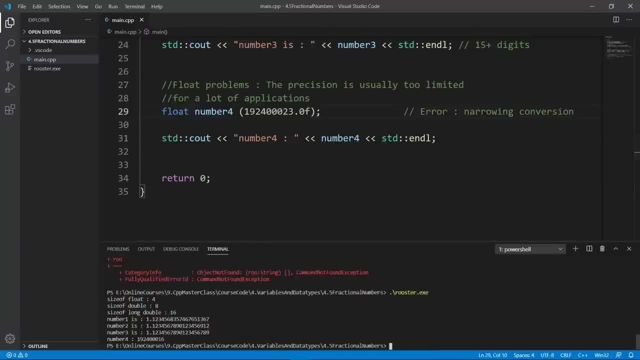 let's run rooster and you see that we get the same results. our 23 is chopped off here. we can also use the assignment notation here, just like we did with integers, and this is going to do exactly the same thing. it is going to chop off the 23 here and we're going to have some. 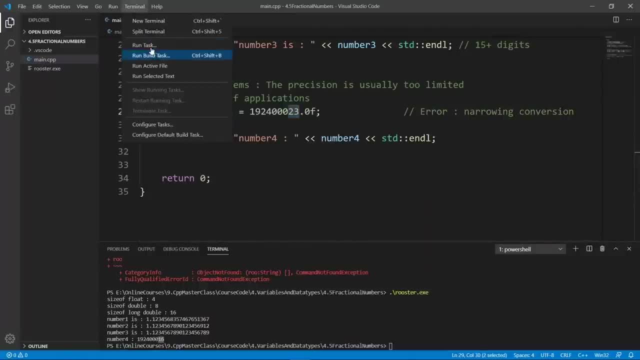 garbage, which is 16 in this case. if we build again, the build is going to go through and if we run, we're going to see a 16 here. okay, narrowing conversions are something you should be aware of when storing your floating point numbers, and you should really remember to put 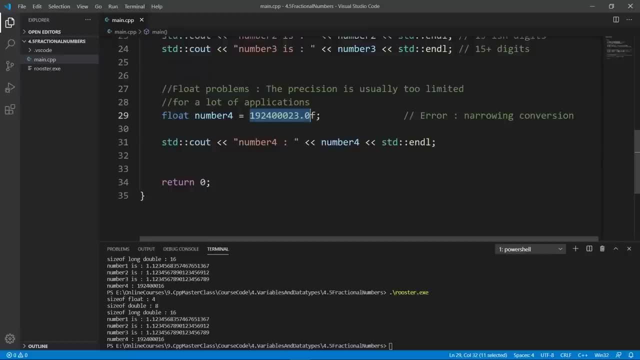 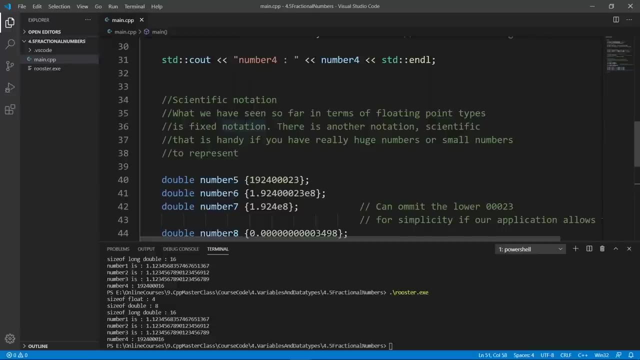 in your suffixes here. and other thing we have seen that we should really play with is scientific notation. as the comment here says, what we have seen so far in floating point numbers is fixed notation. it is what we have here, but we can also use scientific notation. 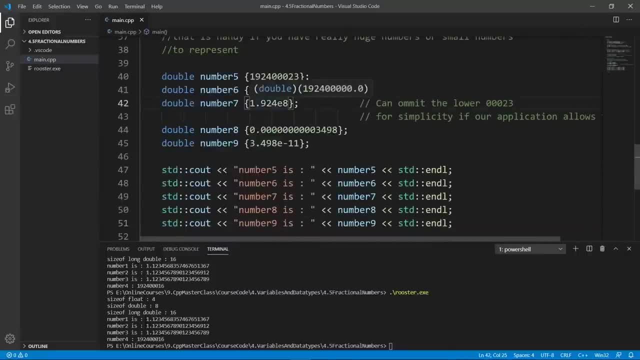 which is exactly what we described in the slides. and what we have here, for example, is e8, and it means that we are going to multiply this number here with 10 to the power of 8.. if you go down here, we have number 9, so we have 3.498 and we have e minus 11, and what this is going to do? 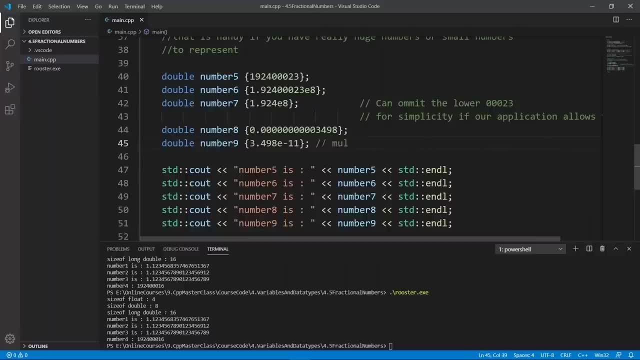 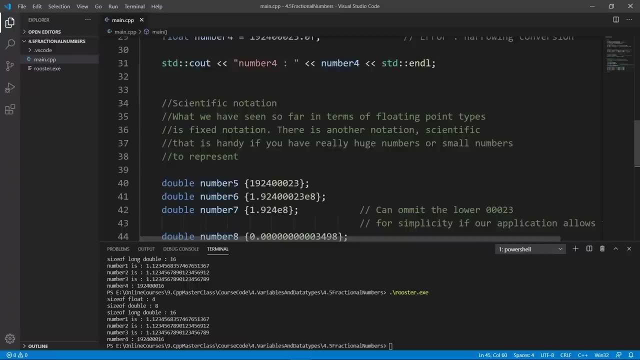 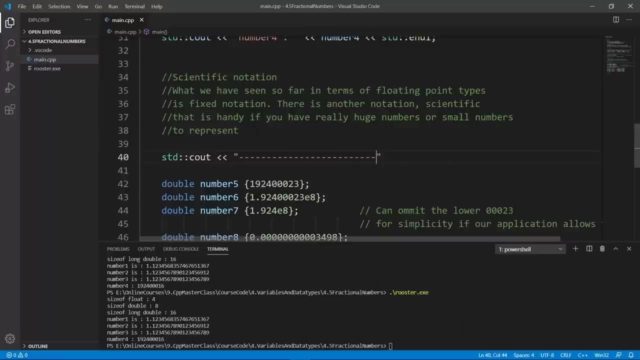 is: multiply with 10 to the power of minus 11.. this is how i can represent this here and we can print these numbers out to really play with them, to make a difference with what we have been doing before. we're going to do, stdc out and put a dividing line here. this is one way we can. 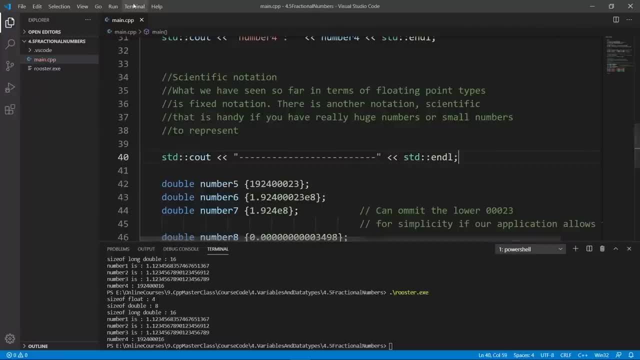 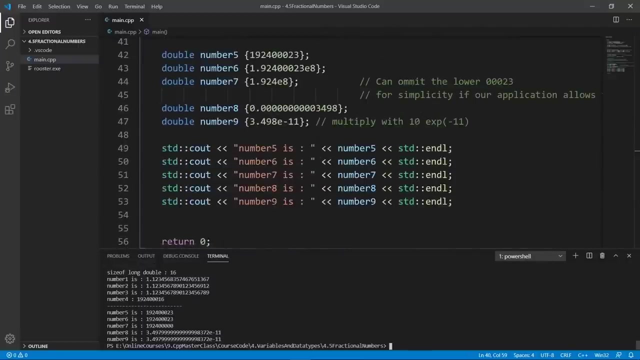 do this, so we're going to do std and dl. we're going to weld this, so we're going to run the tax to world with gcc10. the world is going to go through. if we do rooster, we're going to see that our number here, number five, is what we expect. number six: 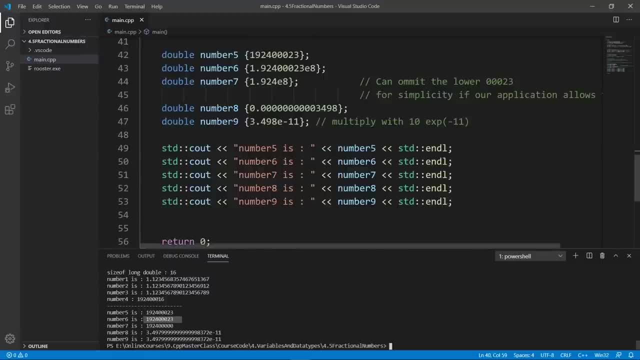 is the same thing, but we used scientific notation to do this, because we took this number and multiplied by 10 to the power of eight. number seven should be almost the same thing, but the lower 23 here is going to be chopped off because we haven't specified it. we're just multiplying. 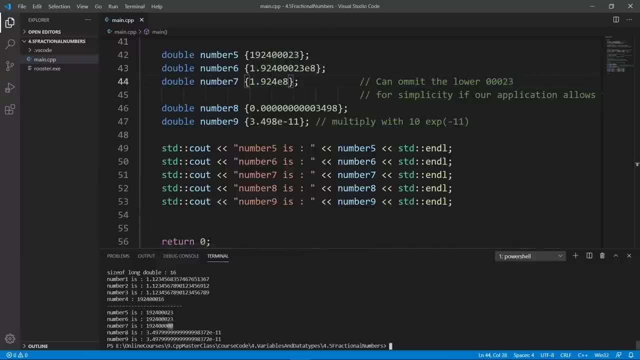 with 10 to the power of eight. so that's why we have zero zero here. i hope that makes sense. and if you look at number eight, you see that we stored it like this, without using scientific notation. we used fixed notation. but on the terminal it's going to be printed out in. 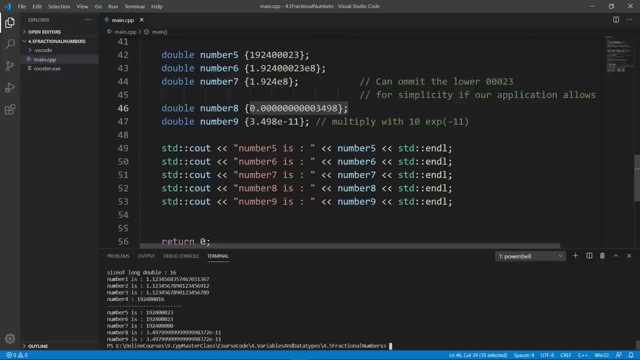 scientific notation, and this may be pretty cool. the main usage for scientific notation is to make sense of numbers that are really huge. so the way you interpret this, you're going to move these numbers after the decimal points with zero in front, and it's basically going to be like this. so if you count the zeros you have here, we're going to have one, two. 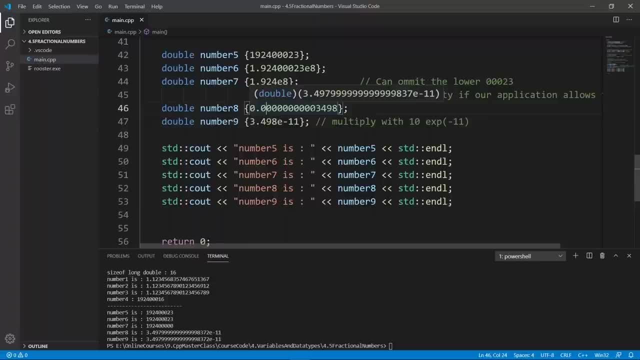 four, five, six, seven, eight, nine, ten and eleven is going to be directly after three and you're going to get the number here. this is what we mean, and number nine was explicitly stored in using scientific notation, and you see that we have the same thing. you can play with these things and 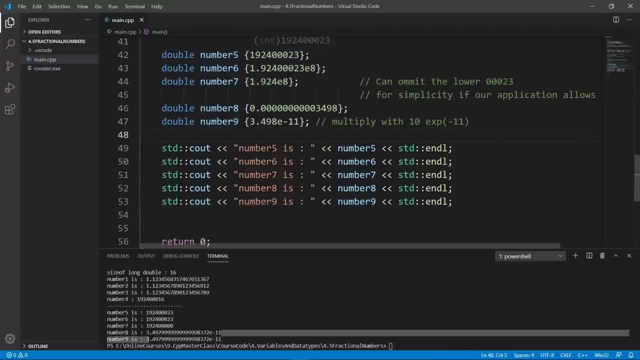 really make sense of them. and again, we didn't specify any suffix here, so these are going to be interpreted as doubles, but this is not a problem because they are doubles here. okay, we are making some progress with this lecture, which is a little lengthy. the last thing we want. 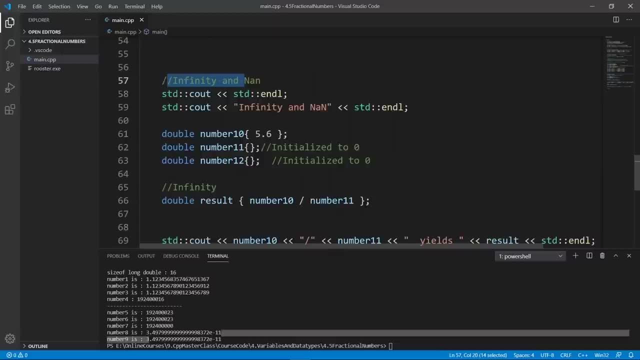 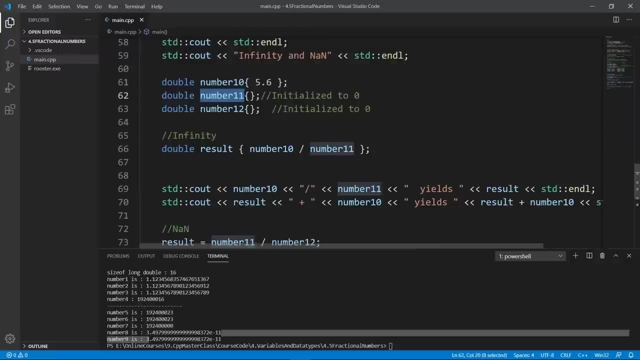 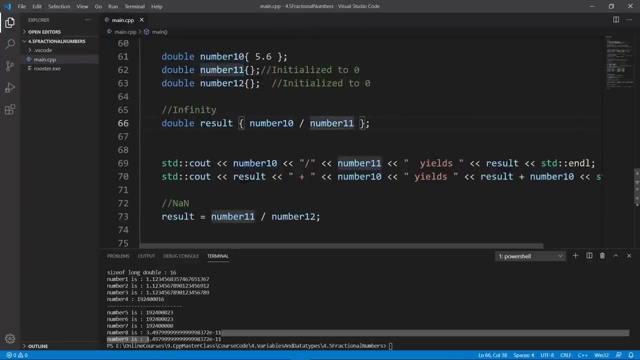 to do is to play with infinity and nan. we're going to put a message here to say what we want to do, and we're going to have number 10, which is going to be positive. we're going to have number 11, which is going to be 0.. number 12 is also going to be 0.. if we take 10 and divide that with 11, we're. 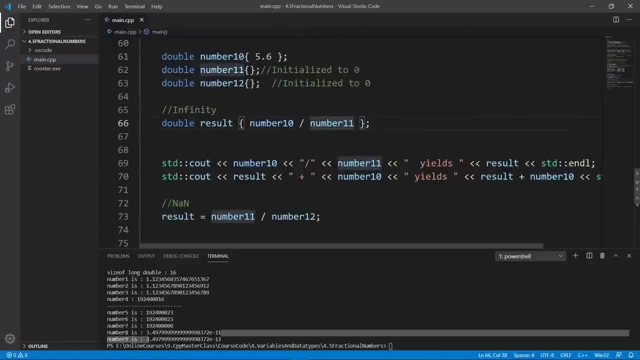 going to get infinity because we are dividing a floating number with 0. if we try to print that, we're going to get infinity. and we're going to get infinity for this result here, because we are trying to add something small to infinity, which is something really big. and if we are trying to 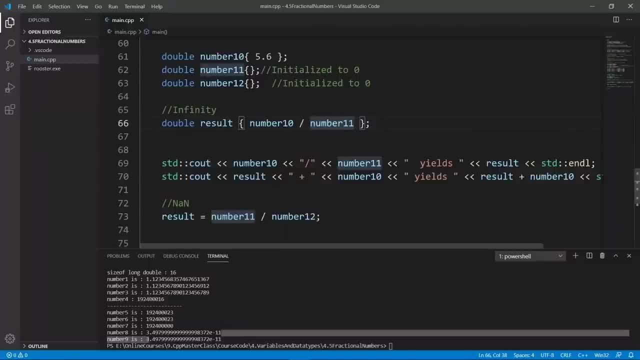 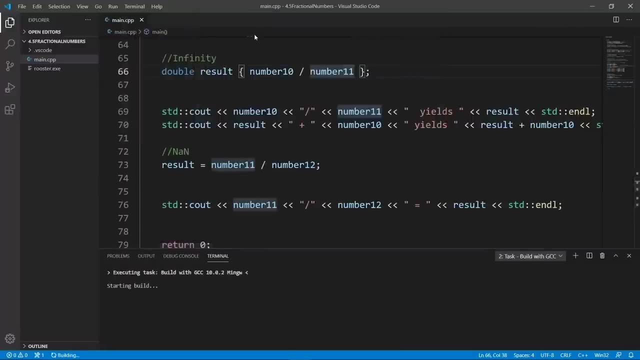 divide 0 with 0 in floating point, we're going to get what is called, not a number, and if we print that out, we're going to see this in a minute. let's build this with gcc. we're going to well successfully. let's clear this out so that we don't have noise in here, and we're going to run. 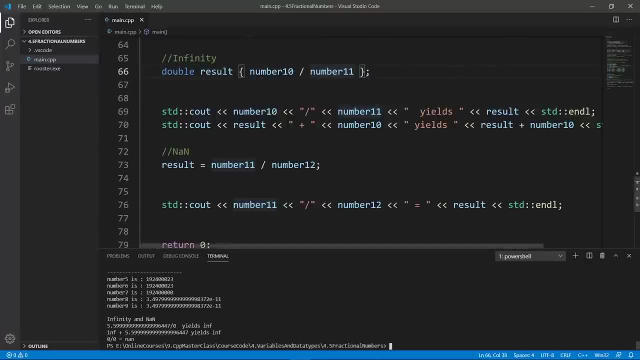 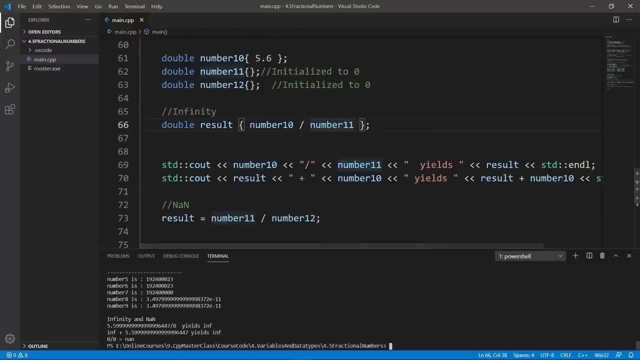 and you see, here it says infinity and none, which is what we said here. and if we go down, here it is saying number 10 divided by number 11, and number 11 is 0. you see that here it's going to yield infinity. if we add 5 to infinity, we're going to get infinity. and if we try to divide a 0 by a 0, 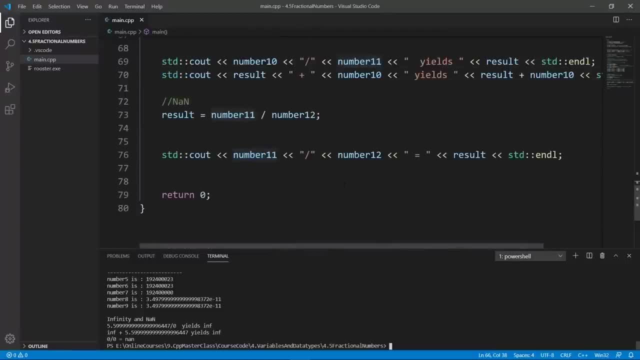 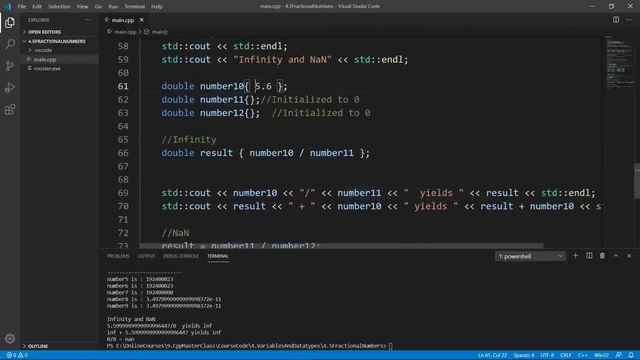 we're going to get none, which is really a way to tell you that you're doing something wrong. you should really be careful. one other thing i want you to see is that if you turn this 5 into a minus 5 and world again, we're going to world. 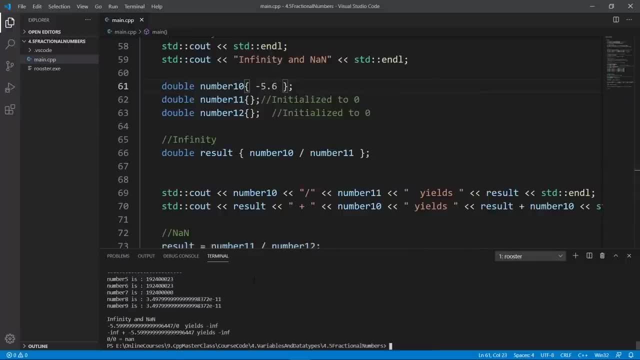 with gcc and we're going to run this rooster, we're going to get minus infinity. so if you divide a positive number with 0, you're going to get positive infinity, and if you divide a negative number with infinity, you're going to get negative infinity. and this is what we see here. this is. 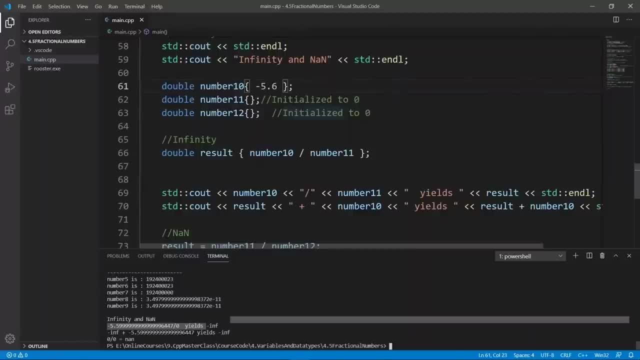 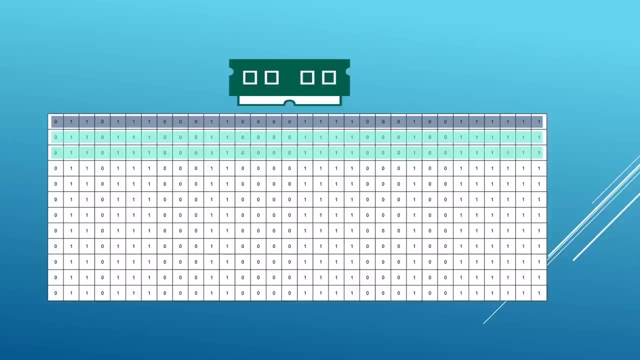 really all we set out to do in this lecture. i hope you found it interesting. and again, the big message here is that if you're going to be handling any data type you're going to be handling in your c plus, plus program is going to ultimately be stored as ones and zeros in memory, and we have 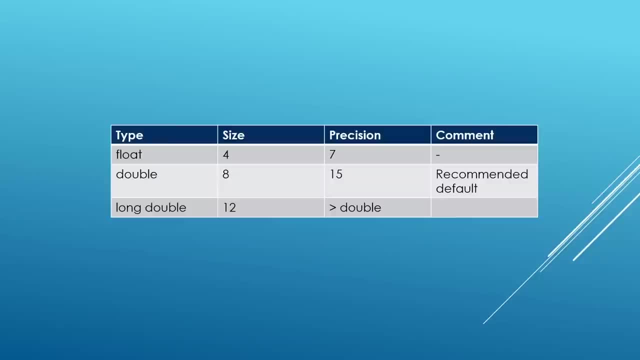 learned about floating point numbers, float double and long, and they have these properties you see here, and you should use them with this in mind, otherwise you're going to have problems with your precision. make sure you are using the correct precision that you need in your program. we are. 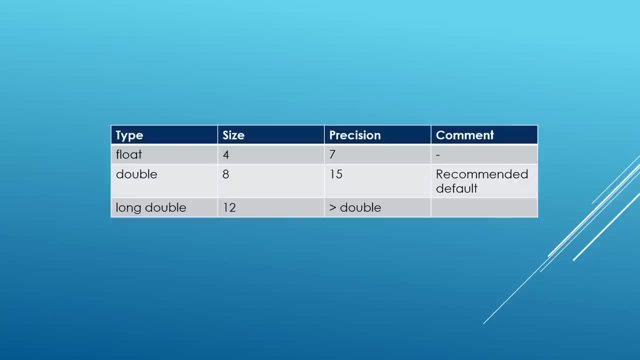 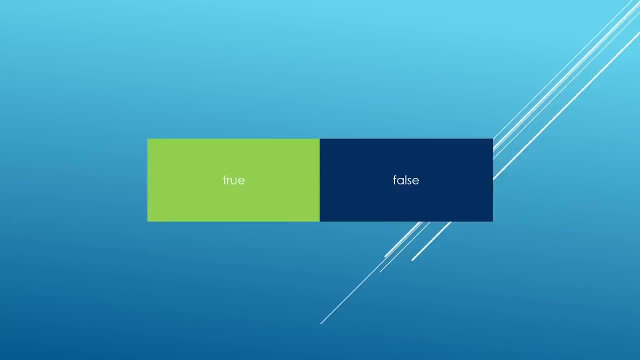 going to stop here in this lecture, the next one we're going to try and learn about. go ahead and finish up here and meet me there. in this lecture, we're going to learn about booleans. booleans are types that can store two states in c plus plus. it can store either true or false. 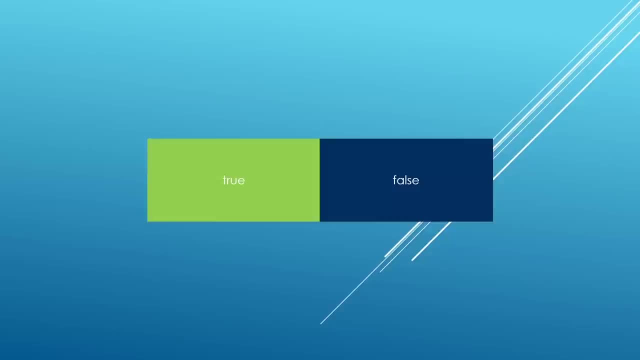 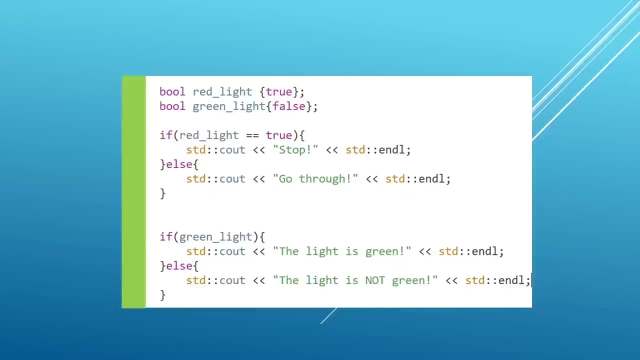 and we can use this to really do decisions in our program. if you look in the program we have here, we have two variables declared, the data type is bull and one is called red light, the other is called green light and we have true and false inside one. 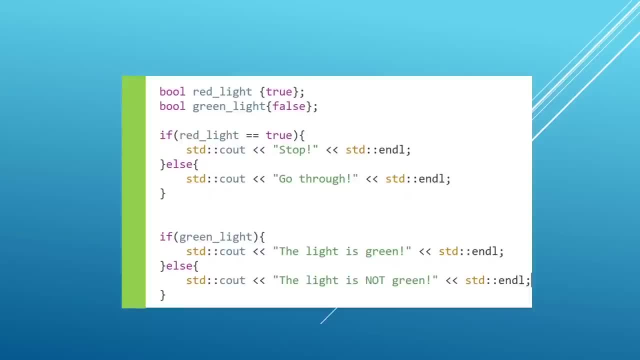 we can do in c plus plus is make decisions. we can say: if the red light is true, we can print a message that says stop, and if it's not red, we can print a message that says go through. we can do that, and booleans are really used in this way: to make decisions in your c plus plus. 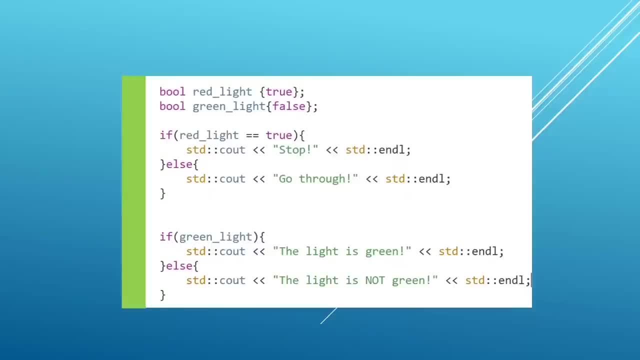 program. we haven't really learned about if statements in this course, but i am throwing this in here to really drive the point home that we can use this to make decisions in our program down here we have another way we can do this. we can actually use the variable. 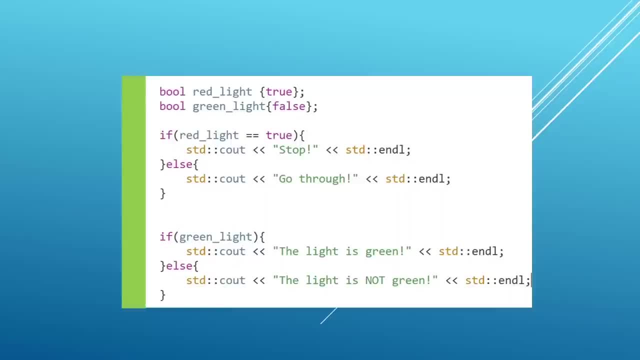 itself, without checking if it is equal to true or false, and we are going to get the same message. the point here is that if green light is true, we're going to say the light is green. if it's not, we're going to say the light is not green. you can do something like this and again. 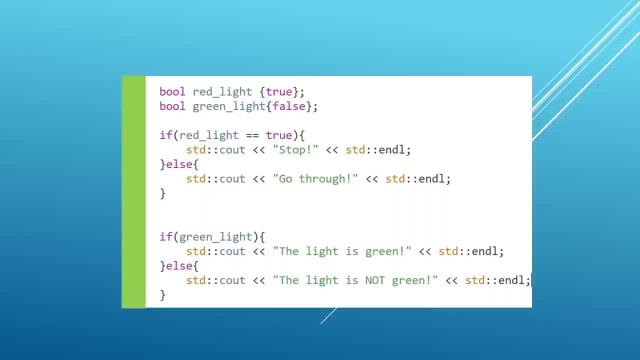 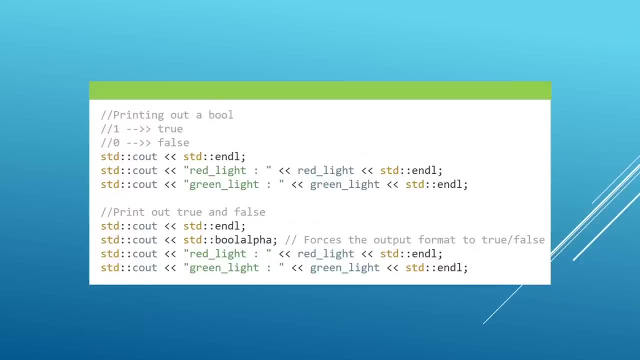 the big point here is that booleans data types are used to store two states- true or false- in your c plus plus program. okay, by default, if you print a boolean that has true in it, you're going to get true, and this is what you see here. and if you print one that has zero in it, you're going to get. 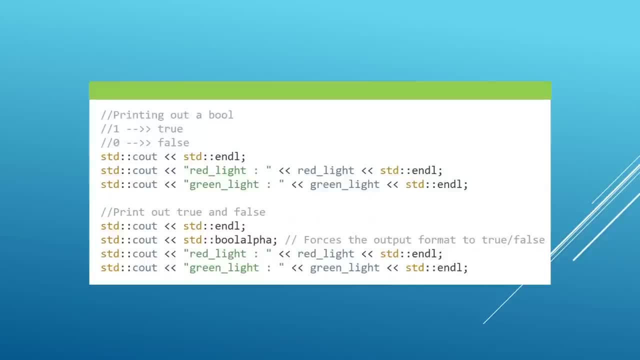 false. we can change that with a special setting that we can apply to our std out stream and you do that like this with std bull alpha and we're going to play with this in a minute. you're going to see if we try to print with this setting applied. we're going to see true on false and not. 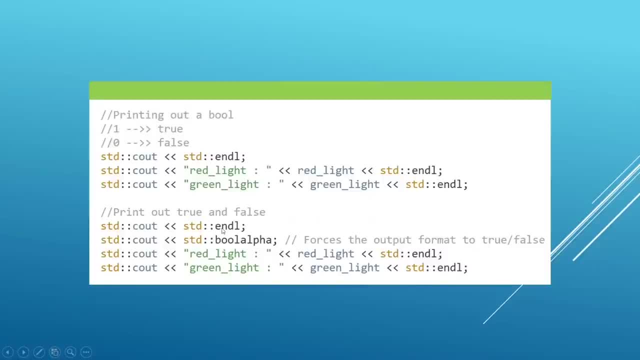 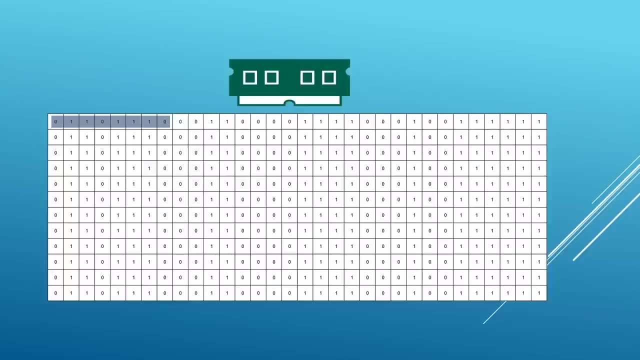 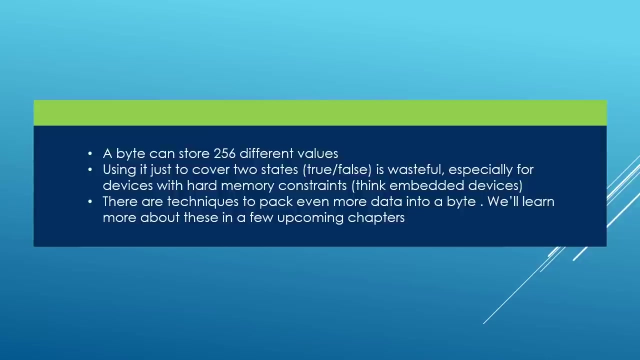 zero and one, like we did before. we're going to play with this in a minute and you're going to see. another thing you should know is that booleans occupy eight bits in memory. they tick up an entire byte. so you may think that this is wasteful, and it is, but with the amount of memory that we have, 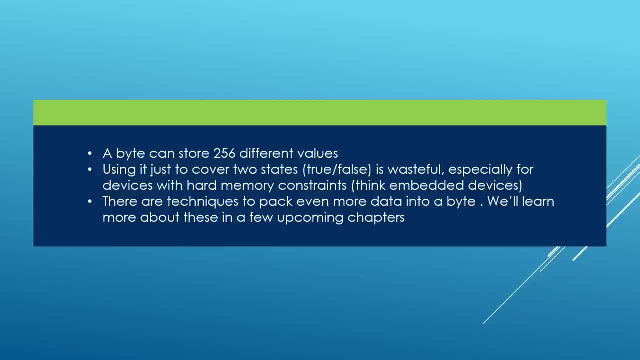 today, this is really not a big problem. but if you are working on a device where memory is really a problem, there are techniques you can use to pack even more data in a byte, and we're going to learn about that later in the course. okay, so this is really all i have to say about booleans. we're 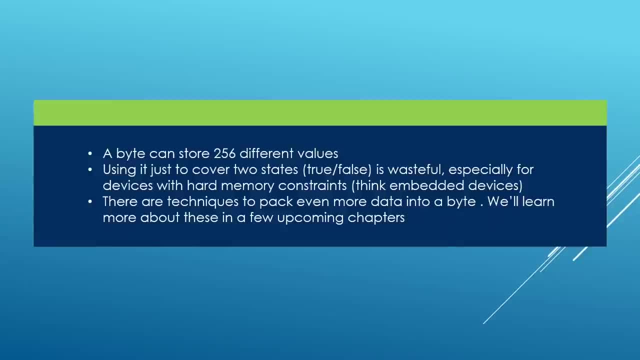 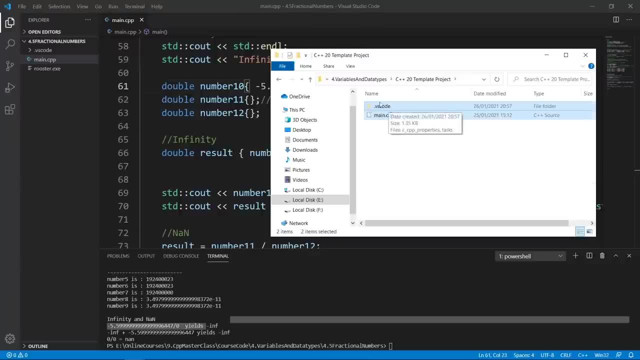 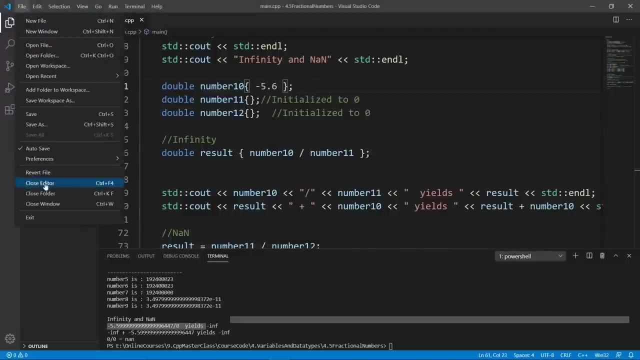 going to go to visual studio code and play with them in code. okay, here i am in the folder for my project. here i am going to do the usual and copy the files over, and i am going to go in my project on booleans. i am going to go up and open this up in visual studio code. i am going to close the. 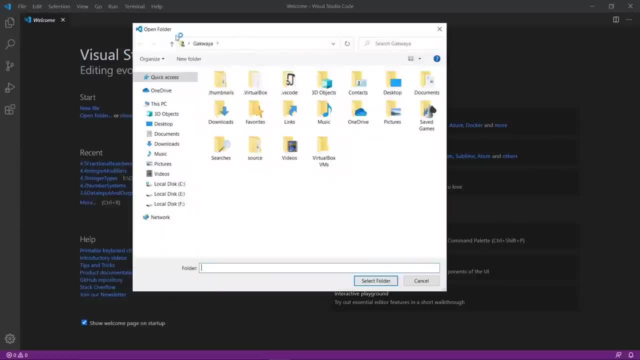 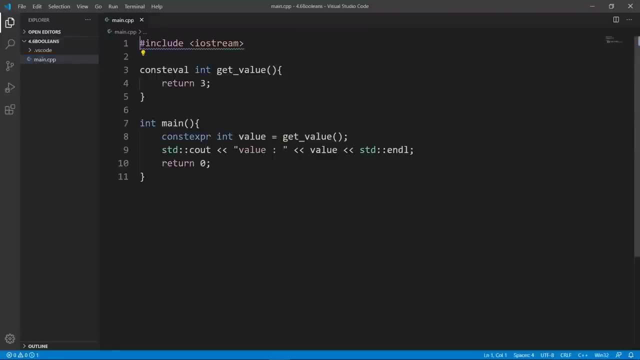 current folder, open the new one and browse to my project. this is going to open up an visual studio code and I am going to close the welcome screen here. I don't need it anymore, so I'm going to remove what I don't need and we are going to. 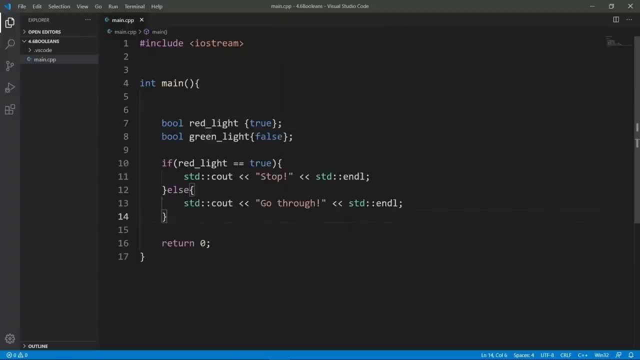 play with the exact code that we had in the slides. we're going to declare two variables: one is going to be red light, the other is going to be green light. they are going to be booleans, and in red light we're going to store a true and 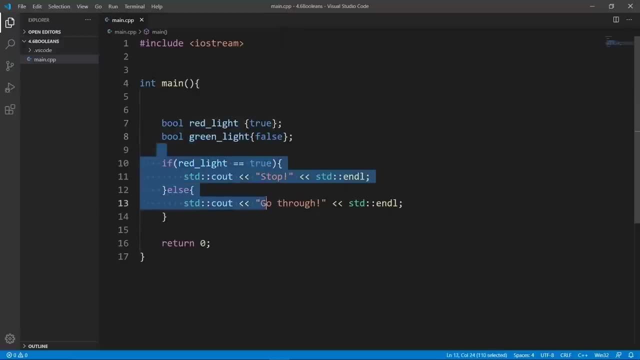 store a false in green light and we can make a decision like this. so try to guess what we're going to print in this program. we're going to try and decide and say, if the red light is true, we're going to print stop. if it's not true. 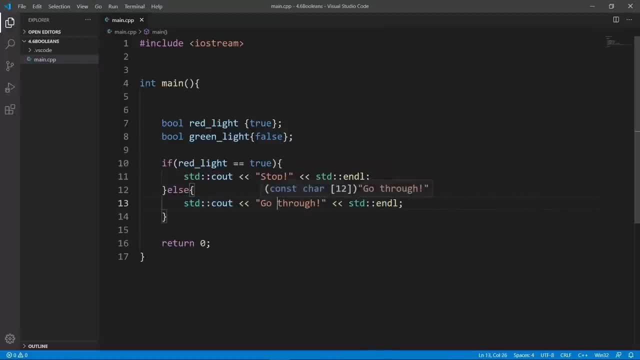 we're going to fall in this block here and say: go through. if we look at our program in red light, we have a true, so this should really win and we should get in this block here. I hope this makes sense, so let's try and build this. 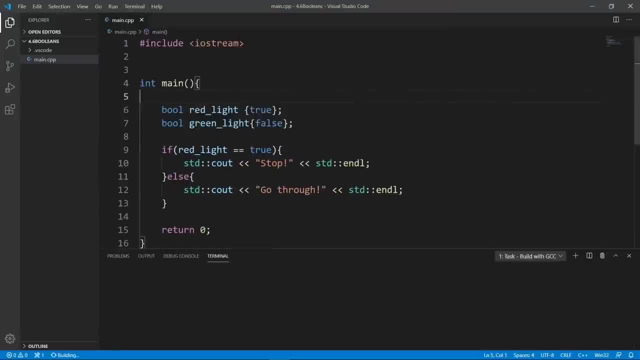 program to see that it actually works. so we're going to build with the GCC, we're going to run our program and our terminal just went away. we're going to create a new one. no big deal, and if we do dir, we're going to see roosterexe. 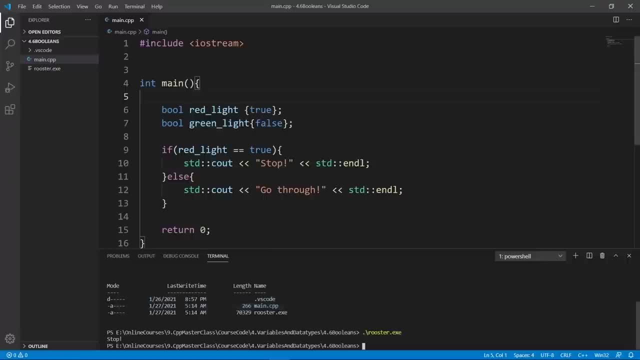 we run it, it's going to say stop. okay, so in red light we have true, the test is going to succeed here and we're going to fall in this block and say stop. I hope this makes sense. you can try to store a false in here and build again going to. 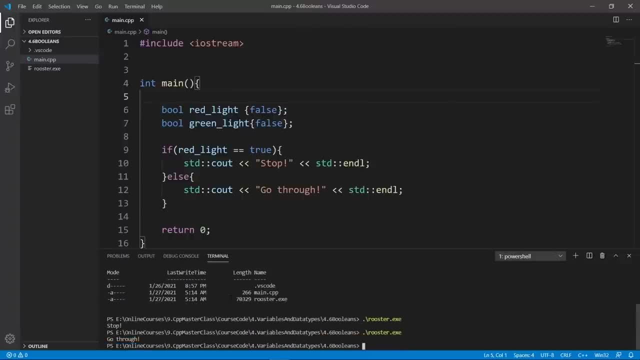 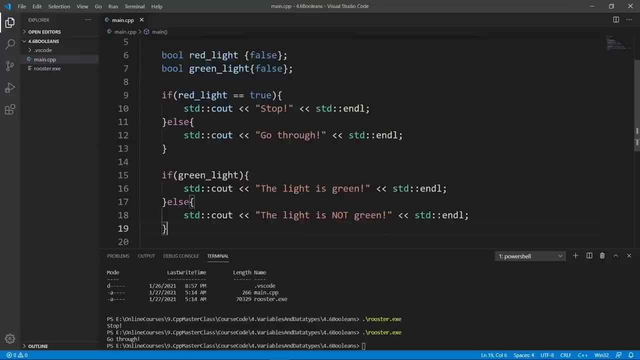 GCC. if we run this program now, it's going to say: go through, because red light is not true anymore. this is really what we mean when we say that we can make decisions based on booleans in our C++ code. we can also try another example. we're going to say: if green light is true, we're going to say: the light is. 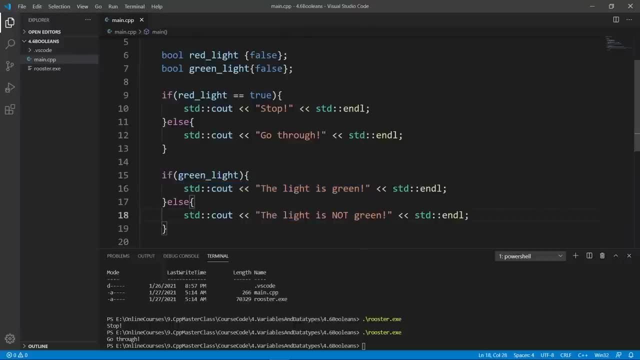 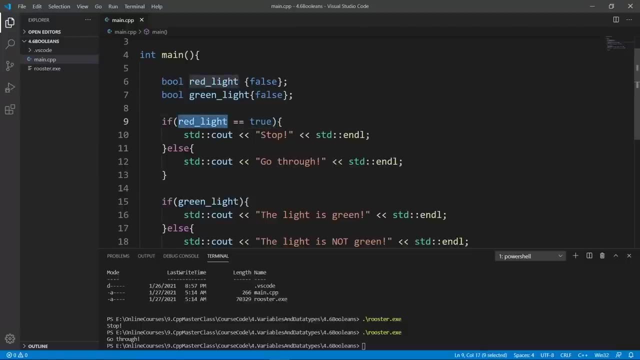 green. if it's not, we're going to say: the light is not green and this is another form we can use instead of typing the entire thing, comparing red light to true here and again. we're going to learn about all these comparisons here. it is just because I thought that talking 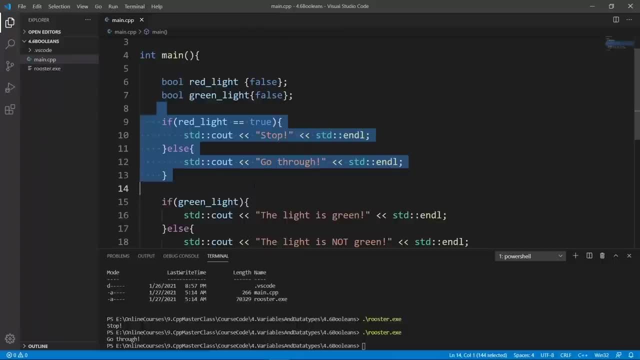 about bulls without showing tests like this is really not going to drive the point home for you. so try to understand this as simple test you can do in math. if one value is true, I am going to do something. if it's not true, I'm going to. 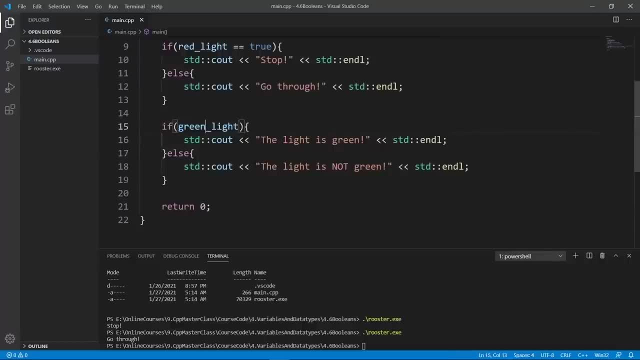 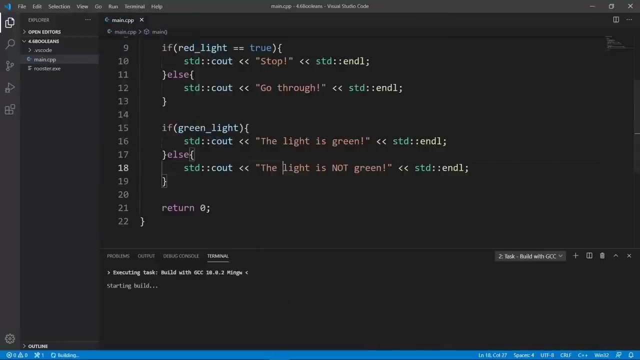 do something else. this is what we are doing here. okay, this program here is: if the green light is true, so we're going to look here. green light is not true, so we should fall here and print this message: that the light is not green. let's build the program. the world is going to go through. we're going to run. 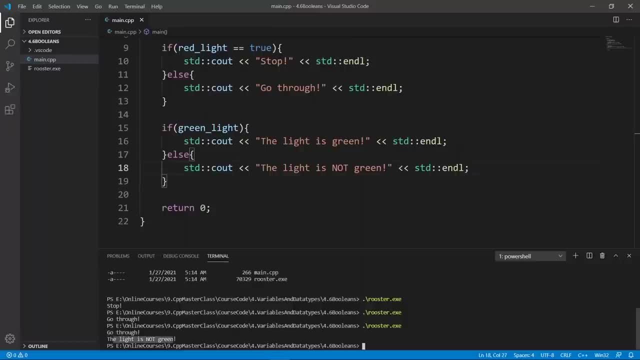 this and you're going to see go through and the light is not green. this is what we have here. another thing we can actually try to see is the amount of memory that a boolean takes up, so we can use size off to do that. we have seen. 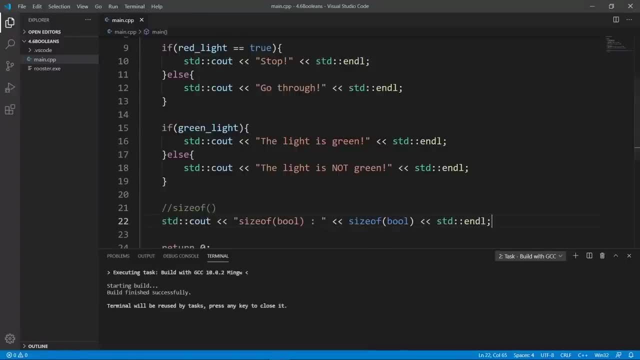 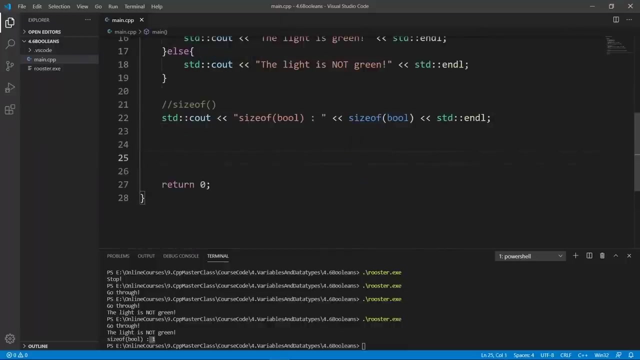 before, if we bought with gcc, we're going to go through and we can run our program to actually this message and you're going to see that ball is actually going to take up one byte in memory. this is what we saw in the slides. another thing that can be really confusing is printing out boolean values, for example. here we 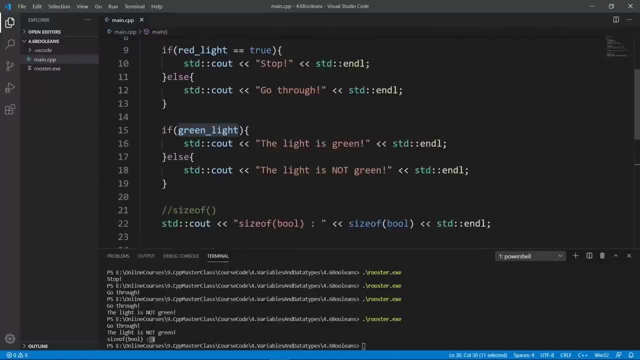 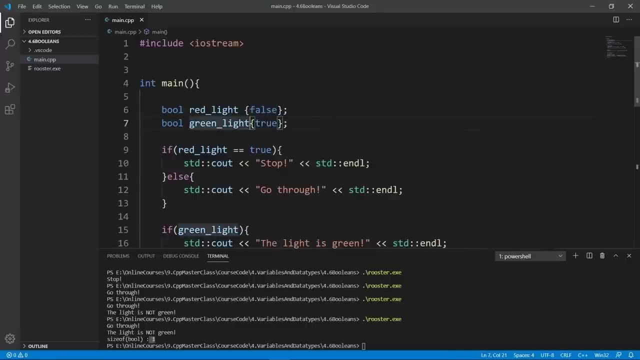 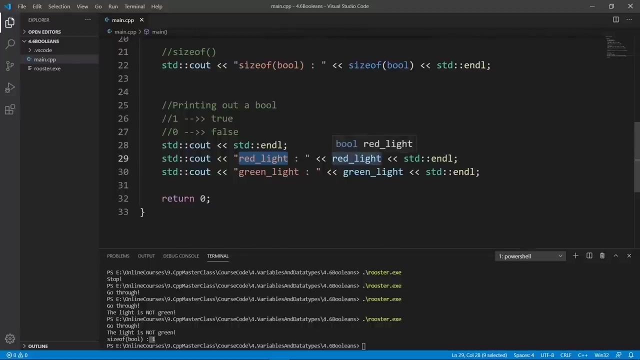 are trying to print red light and green light. let's go up and actually change them a little bit. for example, take green light here and make it true, and we're going to go down again and here we are trying to print them out. red light is going to print whatever value we have stored in, and green light 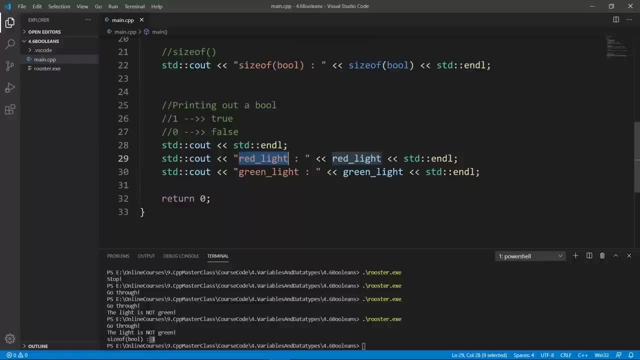 is going to store whatever value we have stored in. and again, true is going to be printed out as one and false is going to be printed out as a zero. let's try and build this. we're going to build with our GCC compiler. the world is going to be. 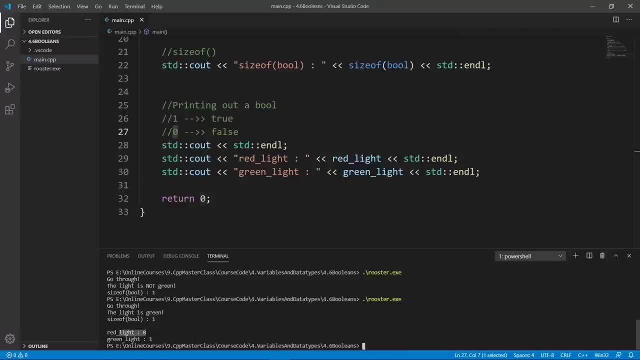 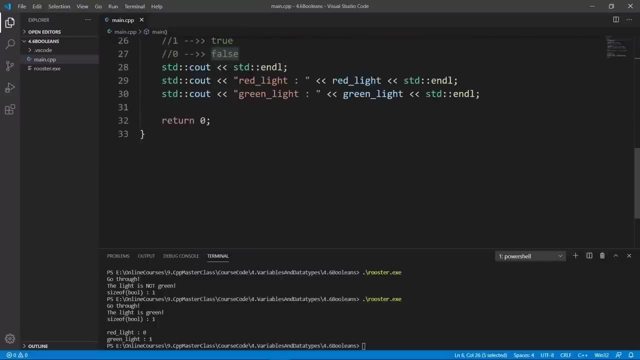 good, we're going to run this and you're going to see that red light is zero because we have a falcon here and green light is going to be one because we haven't a true here. if you're trying to print out boolean variables, you're going 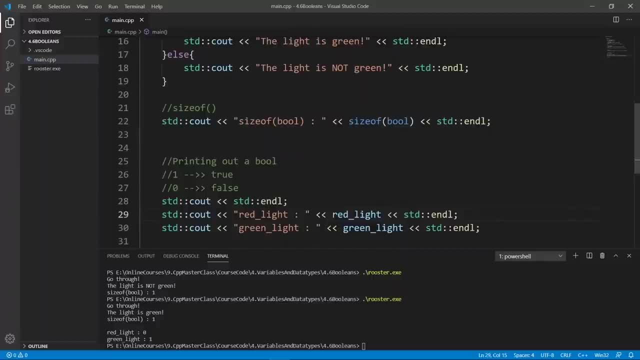 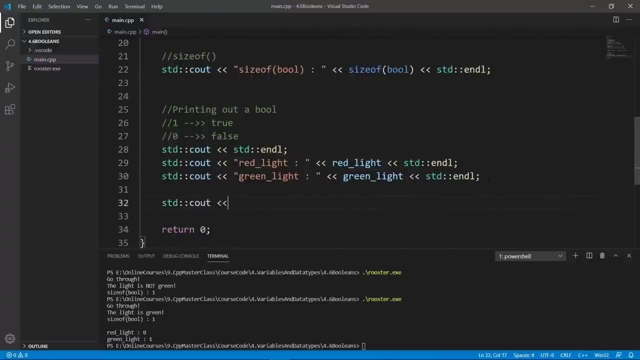 to get one and zero by default. if you really want to see true and false, there is a special setting you can apply to stdc out and you do that by saying stdc out, std bull, Alpha, and you do it like this, and if you print again, we are going to get true and false right now. okay, let's try and 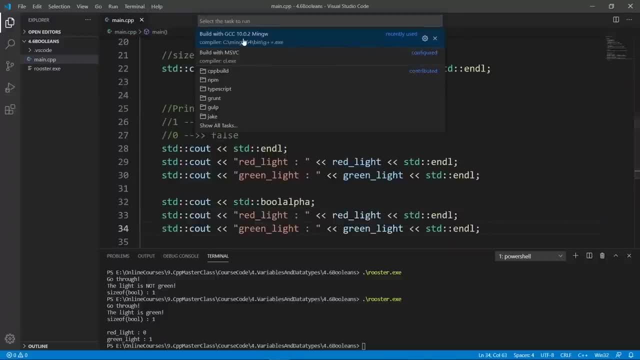 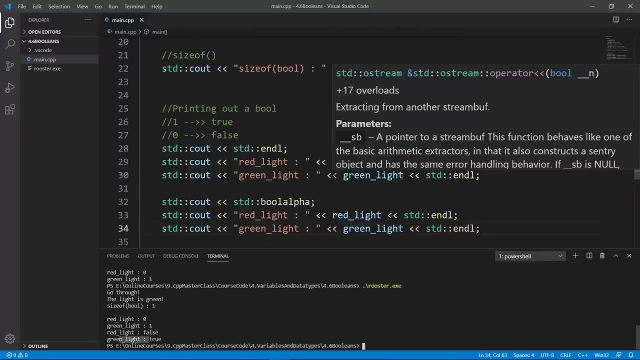 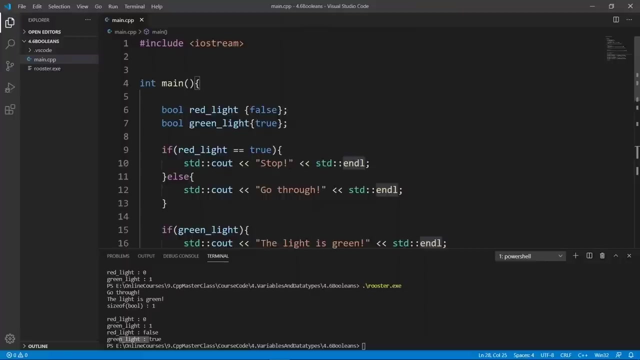 print again and we're going to build this with GCC and we're going to run this, and now you see that we see red light is false, green light is true. this is really all I had to share about booleans in this lecture. I really hope it drives the point home that booleans are mostly used in making decisions in. 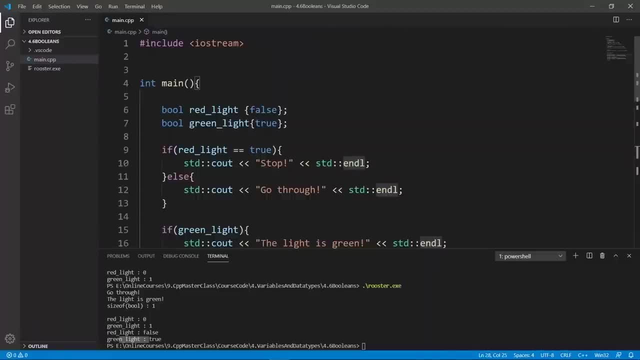 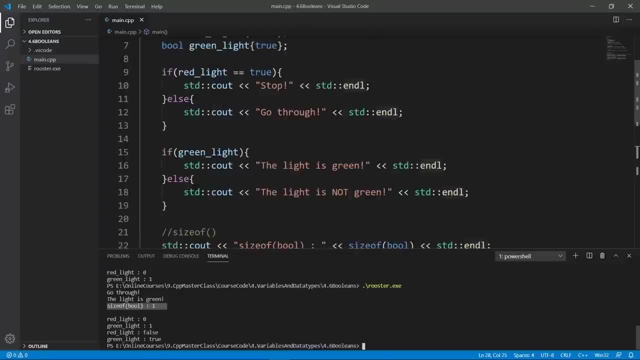 your program and that's what you're going to be mostly using them for. and another thing is that they take up one bite in your memory. we are going to stop here in this lecture. the next one we're going to try and learn about characters and text. go ahead and finish up here and meet me there in this. 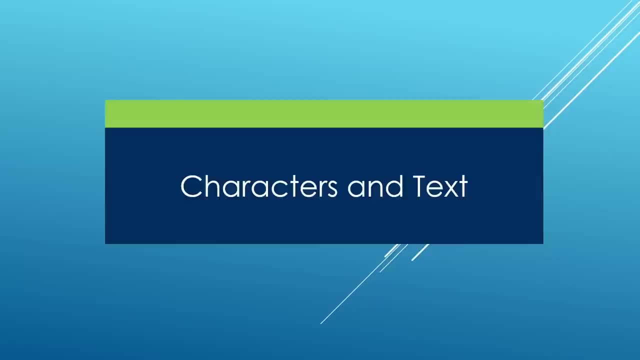 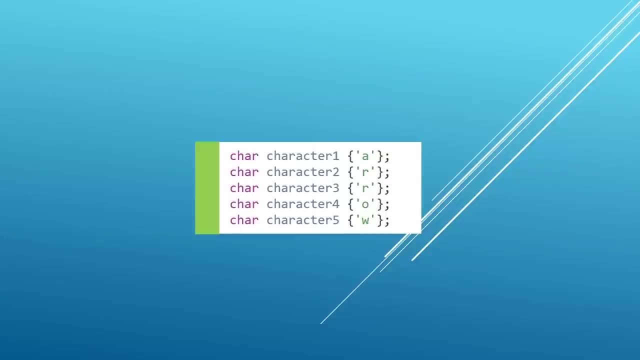 lecture we're going to learn about characters and text, and we use a data type called car in C++ to represent characters, and this is basically how you use it. you store in characters like ABC and here you see that we have a R R O W, and you put your characters in single codes like this to mean that they 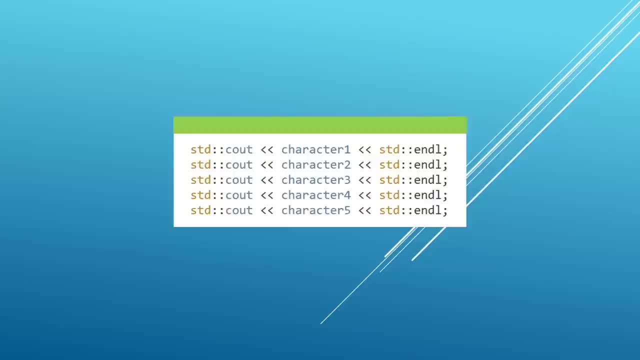 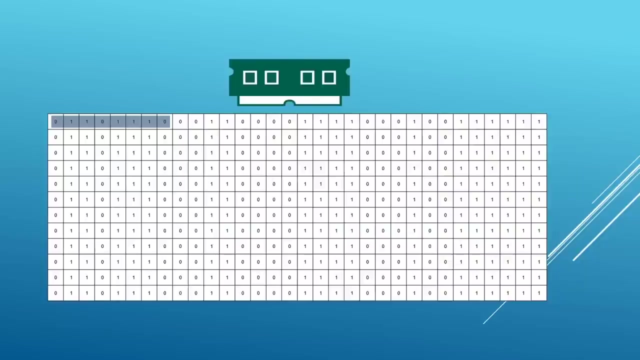 are characters. if you don't do that, you're going to get a compiler error. after you have your characters declared and defined like this, you can print them out with stdc out and we're going to see them on the terminal car occupies one byte in memory, so it's going to take up eight bits. okay, so one thing we can do. 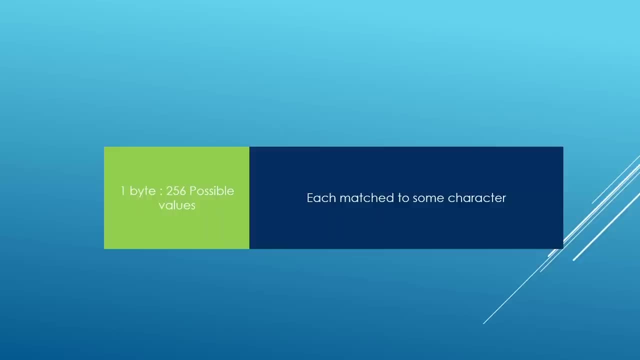 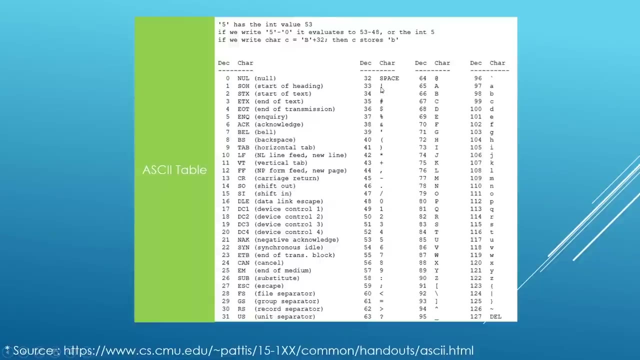 is map each value in these 256 possible values to a character, and we can do something like this. for example, we can say that 33 represents the exclamation mark, 48 represents the character 0, 49 represents the character 1, 50 represents the character 2 and we 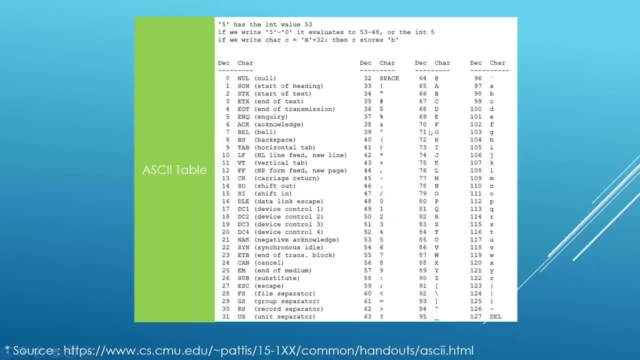 can keep going up and say, for example, 70 represents F, 71 represents G or 100 and 12 represents P. you can really use a mapping like this and come up with representations of your characters in memory, and this is what we do. you can learn about this encoding and on the link here: this is a real thing and it is. 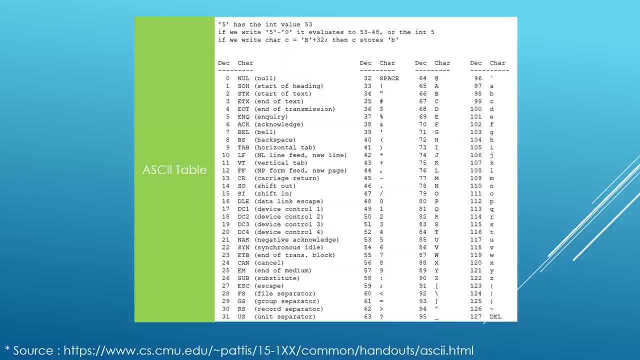 called the ASCII encoding that takes characters and stores them in one byte, and the data type to store these characters in C++ is car. if this doesn't make sense, please bear with me. we're going to play with this in Visual Studio code and it is most probably going to make sense. okay, it is possible. 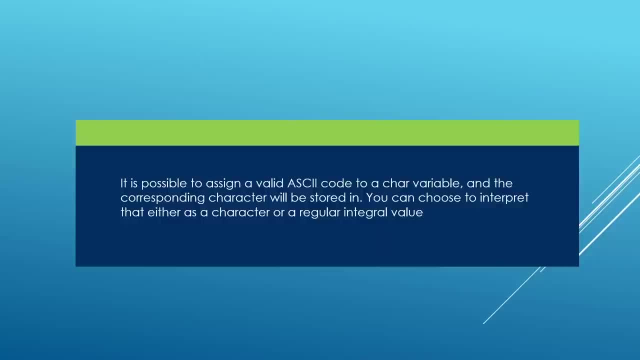 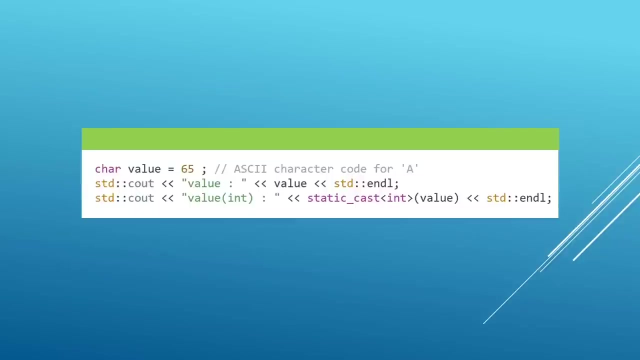 to assign a valid ASCII code to a car variable and the corresponding character will be stored in that piece of memory. so once you have that, you can choose to interpret that either as a character or as a number. that is something like an integer. this is what we really mean if we declare a variable called value, which 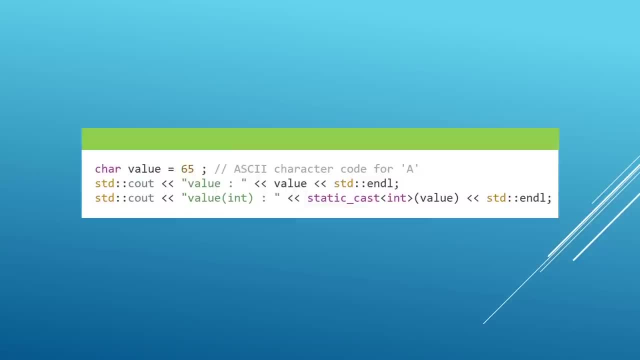 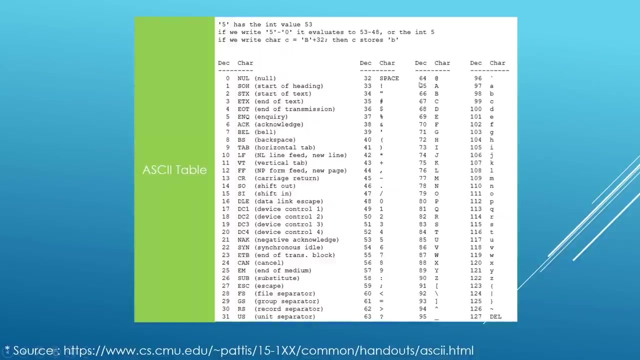 is of car type. a 65 is going to be stored in memory, but the C++ program is going to interpret this as a character. if we go back to our table and see what is represented by 65, this is what we're going to find. we're going to find that 65 represents a and. 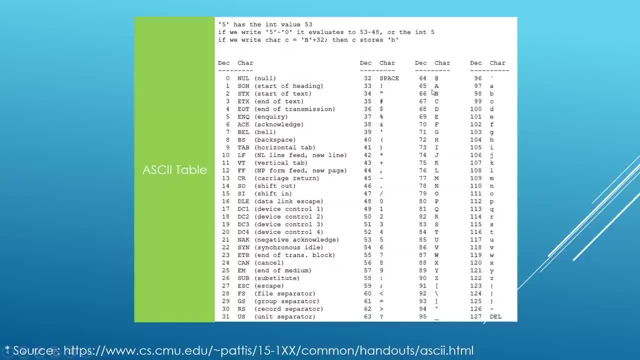 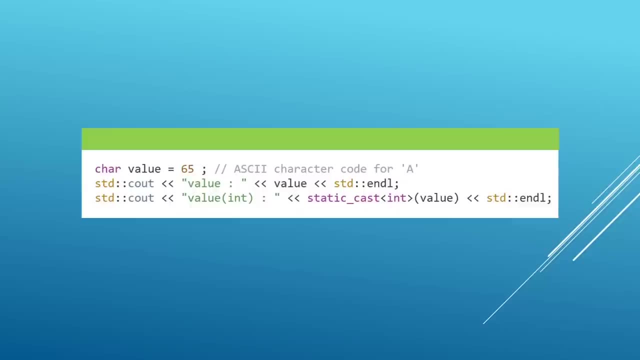 if we print this out, by default it's going to print a, it's not going to print 65.. but there is a way you can take this character value and turn that into an integer and print it out and you see that here we are saying value ant and we 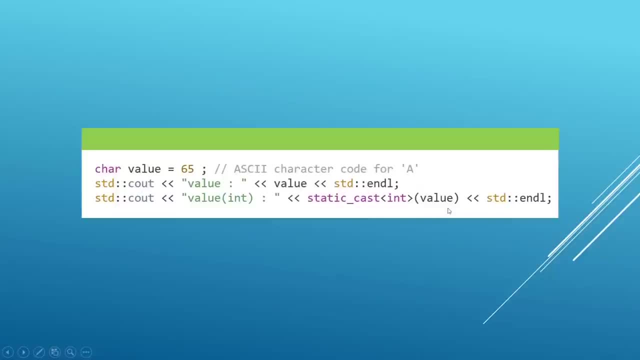 are saying static cast int and parents, we have our value. this is basically a way to say: we want to take the value and interpret that as an integer- and we're going to learn a little more about static cast later in the course- but it is basically a way to 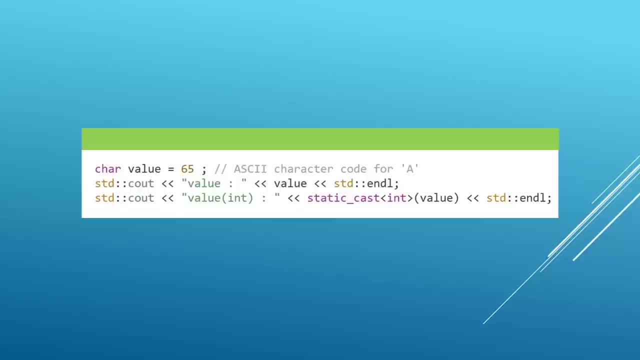 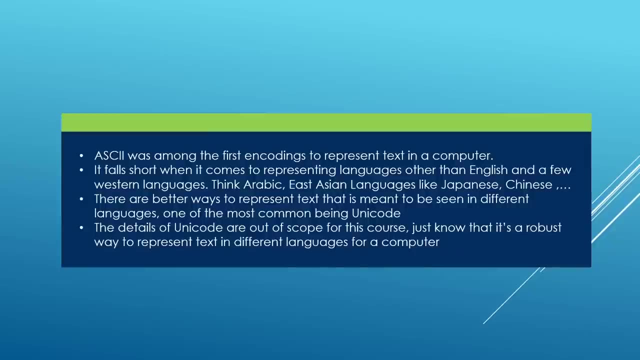 transform between data types and in this case we are trying to transform from car to int and we're going to print this out. okay, what we just described is the ASCII encoding, a technique by which we can map the first 128 numbers in a byte to characters and use that to represent characters. this technique, 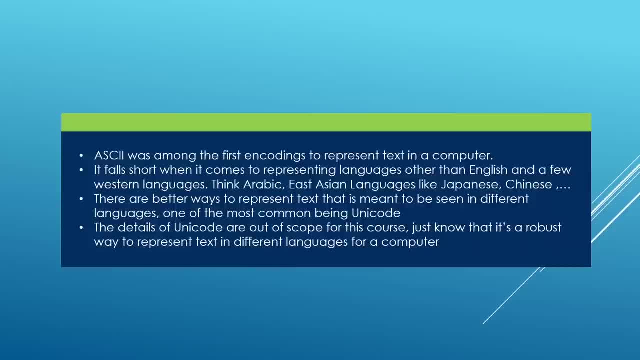 doesn't work well if you have languages like Arabic, Japanese and Chinese, because they are completely different beasts. there are better ways to represent characters in your C++ program, and that's usually Unicode, but that's really out of scope for a course like this, so I'm not going to describe that anymore. 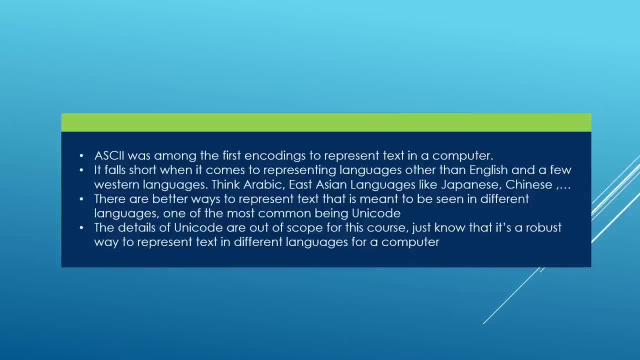 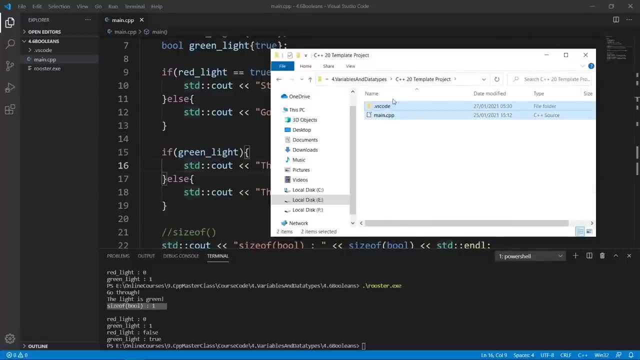 okay, this is really all we need to learn about characters. we're going to head to Visual Studio code and play with them. okay, here I am in my working folder. I am going to go in my template project. I am going to copy things over. I am going to put that in my characters and text. 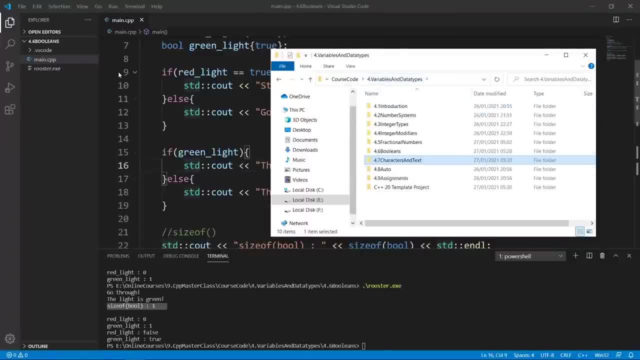 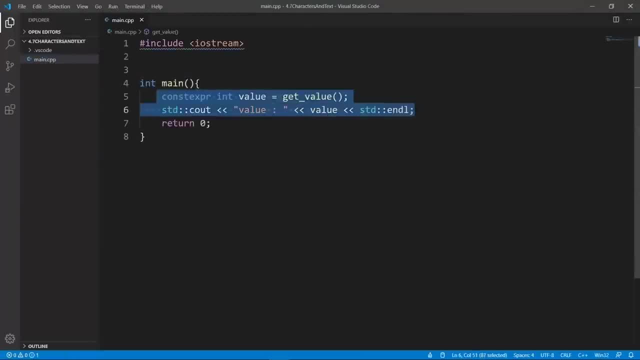 project and I am going to go up and open this up in Visual Studio code. we're going to close the welcome screen here, we're going to open up main CPP and we're going to put in the code to play with characters and text. the first thing we 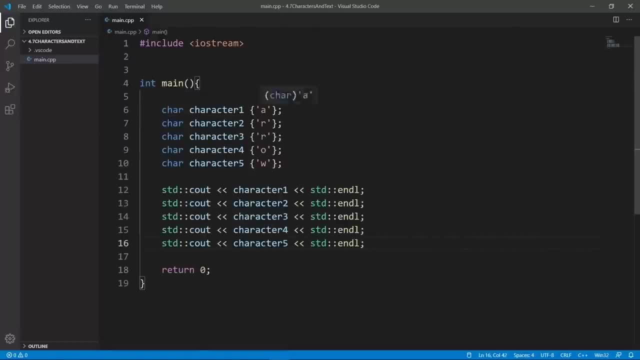 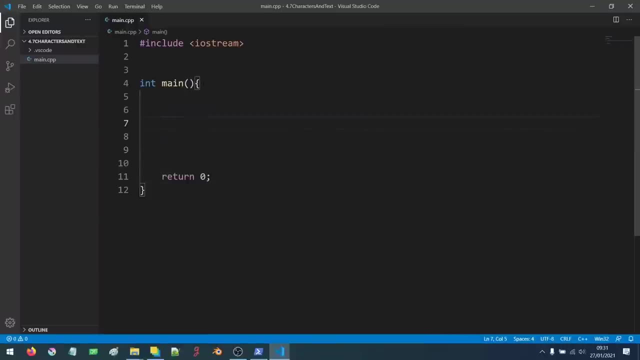 can do is declare characters like this. we can put in a R R R O W here and we're going to see this printed out. if we run this program, we are going to put in some code to play with characters. we have a few variables declared that are of car type. we go from character one through character five and 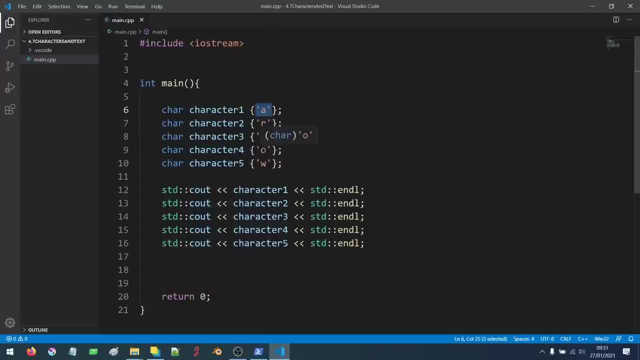 these are the characters we are storing and this is- and this is the format you're really going to use to declare your characters. after we have them declared, we can print them out like we print any other variable, and we can try and compile this program and see what we're going to get. but 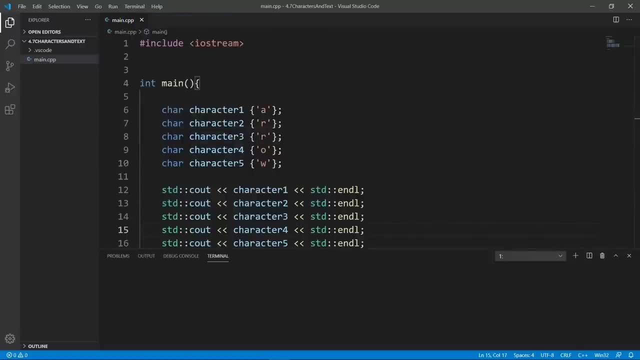 before we do that, I would invite you to try and guess. so let's open our terminal and we're going to build with our GCC task, we're going to build, the build is going to go through and if we run rooster, we're going to see that we are. 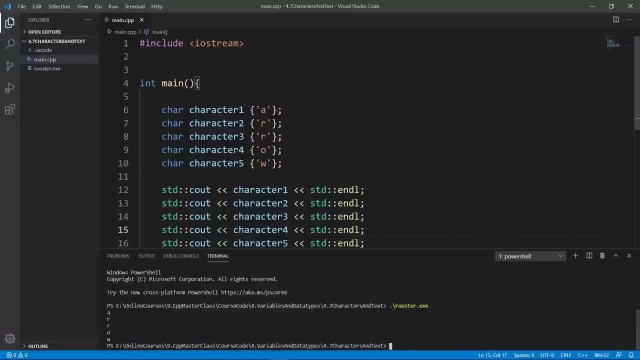 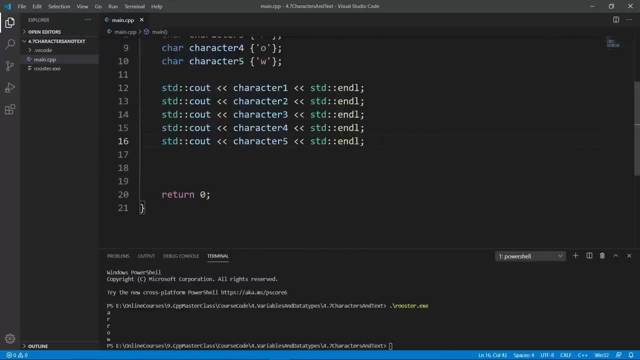 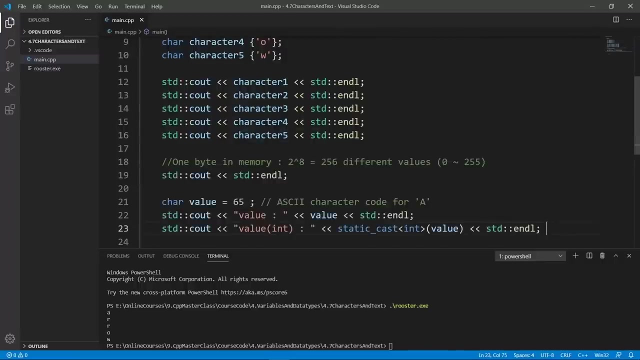 printing out A R R? O? W. we are storing our characters and and we are able to print them out. this is really how you work with these guys. another thing I want you to see is the size that a character occupies in memory. by that I mean car type. it's going to occupy one byte in memory and that means 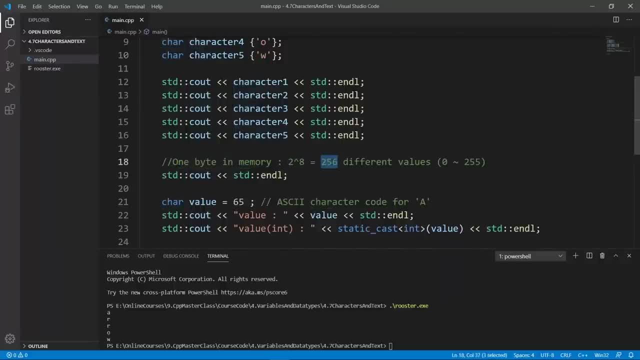 that we can only have 256 different values that go between 0 and 255. if we have decided to store in positive numbers, we are using the knowledge we learned from the integers lecture. if these calculations we are doing here don't make sense, please go back and check that out. so down here we are declaring a character. 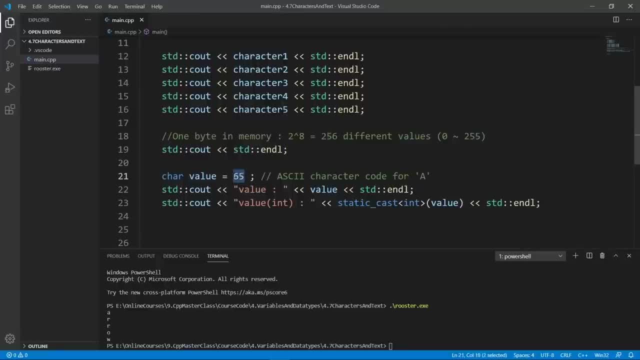 type, the name is value and we are putting in is 65. the thing is, if you try to print this value here, it's not going to print 65, it's going to print a, which is a character representation of 65. if you remember from our ASCII table, we had 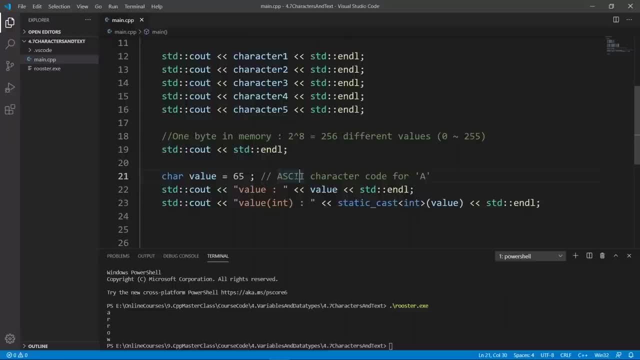 these mappings between characters and integers and 65 mapped to the character A R R O W. so it means that we're going to put in the number of characters and indexes as in between intercontinental number and we we are hoping that then we pass this value that had kept in guiding it when we areREFRGO: individual key. 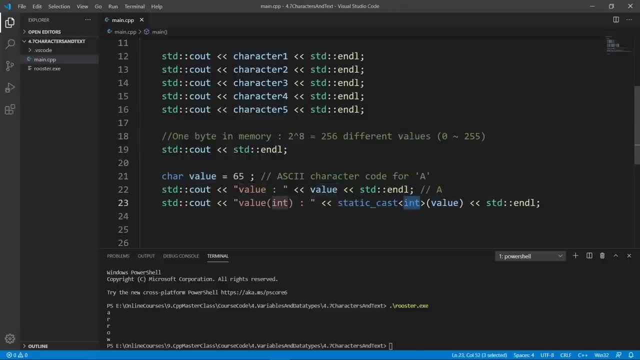 properties, because we do not want to printそれでは set of a cloud and this values is going to be pain 400x. who wants to be able to show results? and this is what happens. when i say that sometimes, very, we opt out of the template, for example, our customers will point to a word: pass. 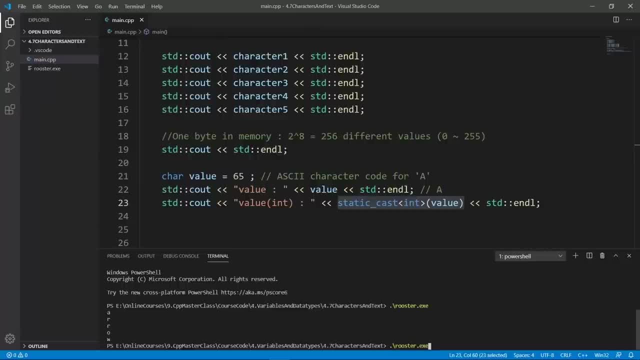 to us. thank désert pro keys a percase. so if we print this out, this is going to give us 8, but we going to see that value is a for the first line here and a value at is 65, because we decided to interpret whatever is in this value as an integer and not as a character, as it is done. 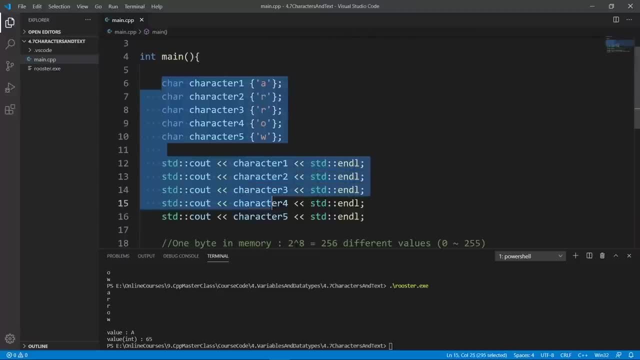 by default. this is really all we set out to do in this lecture. i hope you found it interesting. we are going to stop here in this lecture. in the next one we're going to try and learn about the auto keyword in c plus plus. go ahead and finish up here and meet me there in this lecture. 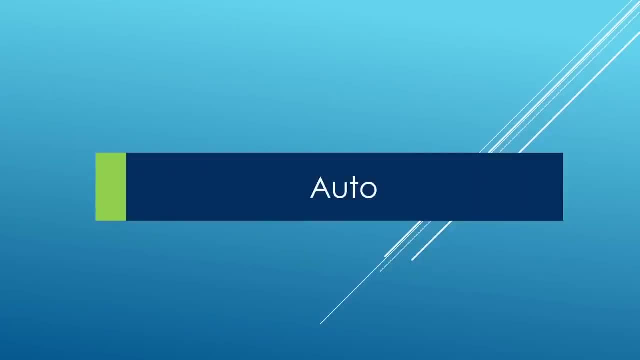 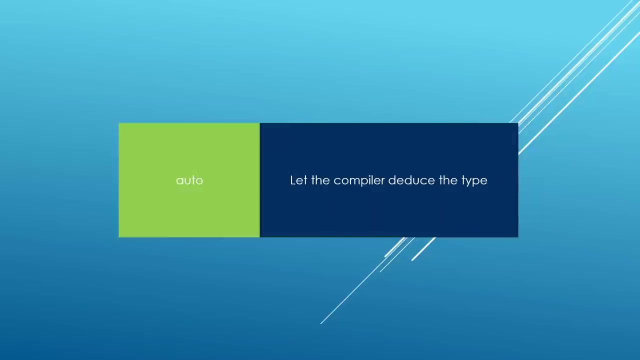 we're going to learn about the auto keyword in c plus plus. this is a keyword that is going to let the compiler deduce the type for you, and this is going to come in handy when you have longer type names that are really hard to type. we can't really give you an example of that because that 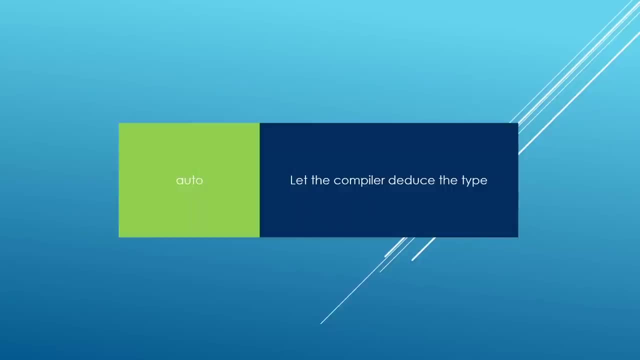 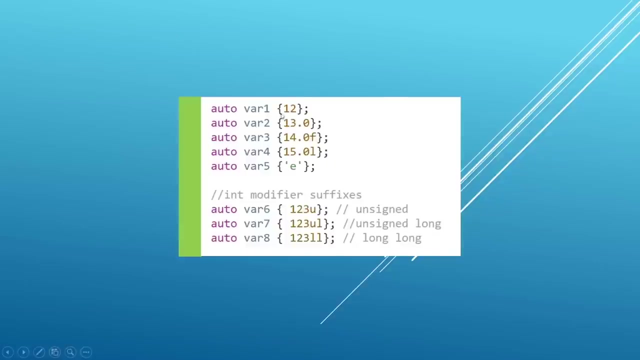 requires to have a good number of concepts mastered in c plus plus. but we are mentioning this here for completeness, because we are talking about variables and data types. so let's hear how we can use this here. we have an example where we are saying auto var 1 and what we initialize this with is an integer. so 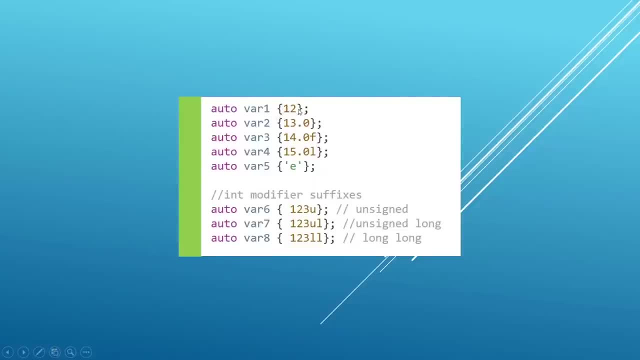 the compiler is really going to try and guess the type of this thing and that's the type it's going to assign to variable one. this is what auto is really used for. if we pass a double inside, and it is a double because we have no suffix here, so it is going to deduce a double. 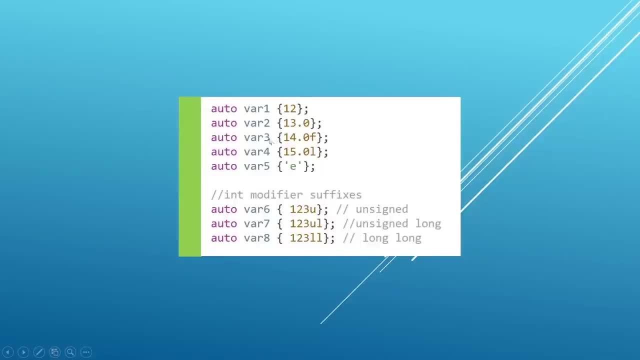 if we pass a suffix of f, it is going to interpret this as a float. if we pass l, it is going to interpret this as long double. and if we pass in a character, it's going to interpret this as a character. and this is really the essence of what auto is used for. it is used when you 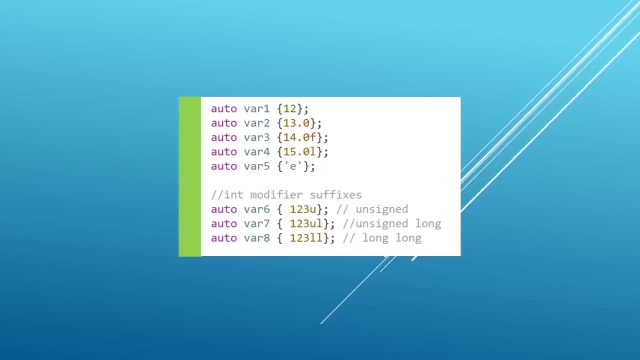 don't really want to你真的不想想起 good exam of what also is used for. when you don't really want to garage, really want to, you know, Pass a character And this is the recipe of what auto is used for. so explicitly type the type of your variable and you want the compiler to fill in that for you. 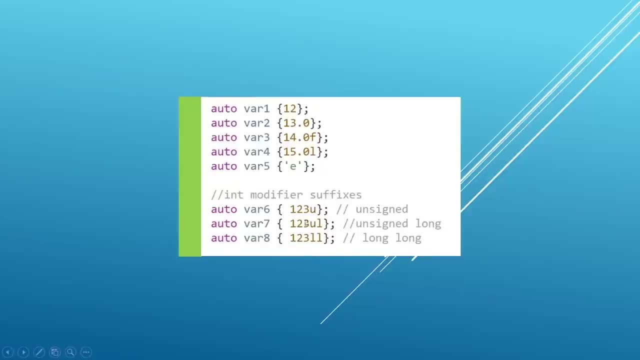 or guess it for you. down here you see that we have a few examples with integers so we can make this unsigned long through these suffixes and the compiler is going to deduce the type based on what we pass in our initializer here down here you see that we have a few examples. 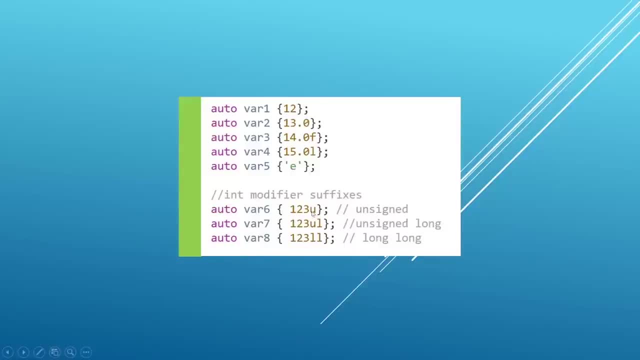 with integers. if we pass a suffix of u, this means that we are storing an unsigned integer. so that's what the compiler is going to deduce. if we pass ul, it is going to be unsigned long. if we pass in ll, this is going to be long, long and that's what the compiler is going to deduce here. you see that we. 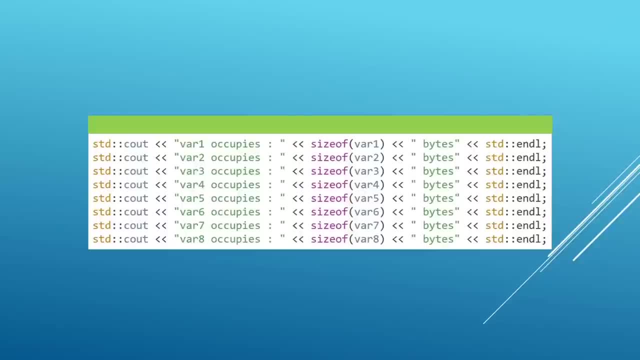 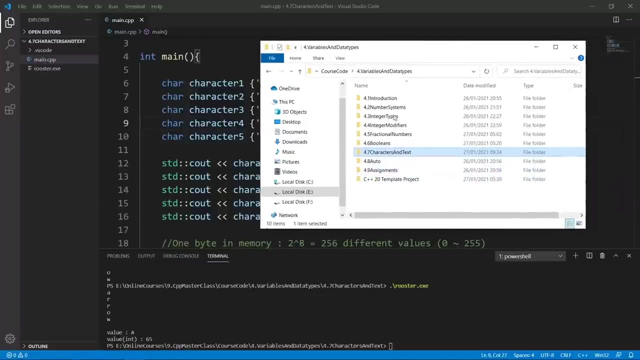 are trying to print the sizes of these variables and we trying to prove to ourselves that the compiler deduced the right size, and we are going to go to visual studio code and actually try this out. okay, here i am in my working folder, i am going to open my template project, i'm going to copy that and i'm going to save my files. 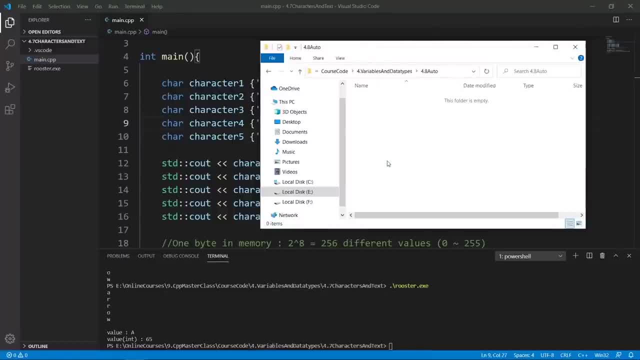 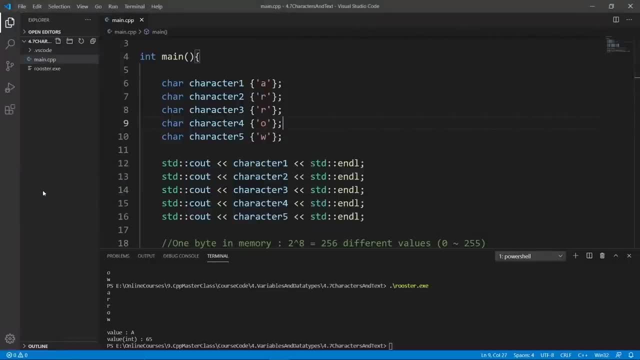 in the auto project here. so i am going to go in and put in my files. i'm going to go up again and i am going to close whatever it is i have in visual studio code because we're going to create a new project. i am going to 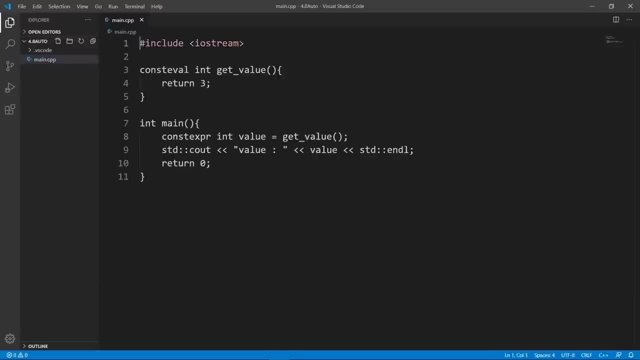 open my new folder. we're going to close the welcome screen here and we're going to remove whatever it is we don't need for this project and we are going to put in the code we basically had in the slides. i am pasting this code in to save on some time because i don't want you to see me type. 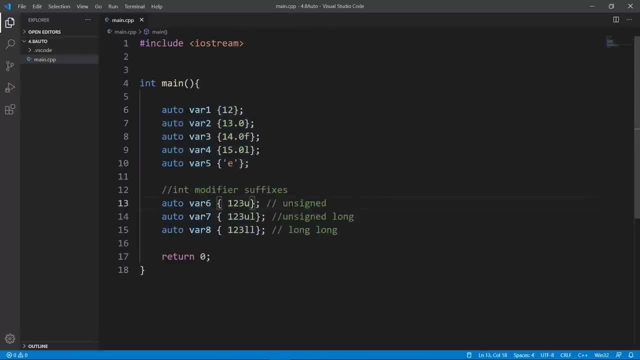 these things. we're going to save some seconds here. so the first statement here declares a variable, var1, the type we don't really know, but we're going to let the compiler deduce that for us. this is the that for us and we can try and actually hover over this, and we're going to see that the compiler 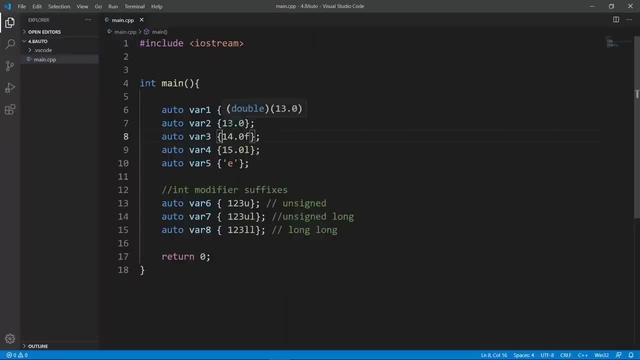 already deduced that this is an integer. if we go to var 2, this is a double. if we go to var 3, you see it's a float. if you go to var 4, it's long double. if you go to var 5, it's a character you. 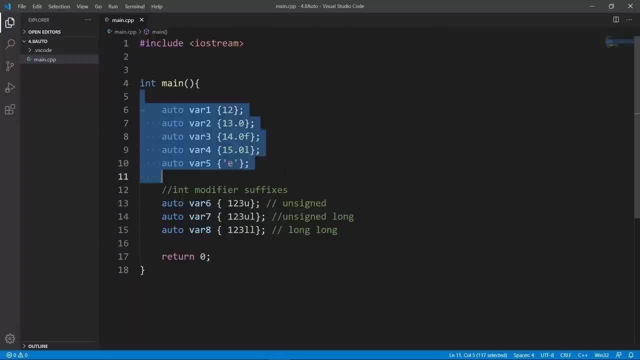 can see that visual studio code can even see what the compiler is going to deduce before we even compile the code. this is the beauty of visual studio code. we're going to look at var 6. you're going to see that it's going to be unsigned. and if we go to var 7, it's going to be unsigned long. 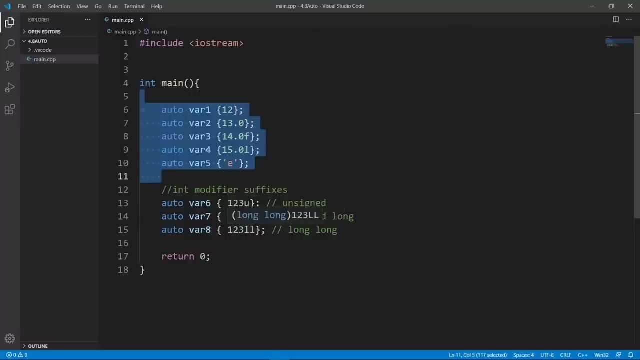 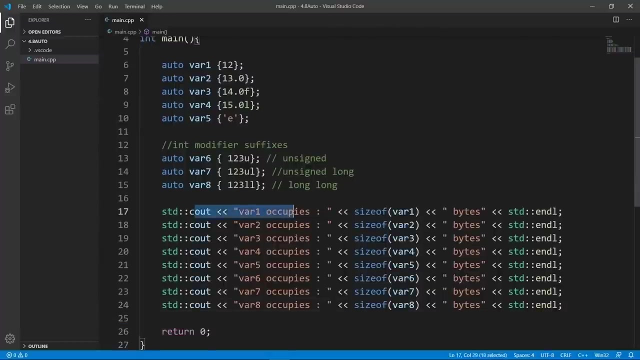 if we go to var 8, it's going to be long, long. this is really cool and you can see that our types are correctly deduced. visual studio code was really helpful in showing us these types, but we want to be sure by running this piece of code and seeing whatever. 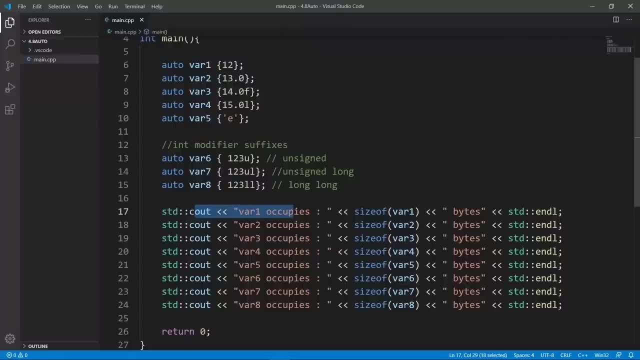 situation we're in. we're going to be able to see that the compiler is going to be unsigned size. the deduced type is, for example, for var 1. we guessed that it's going to deduce an int, so it better be a 4 in size. we're going to try and run this. we're going to open our terminal here. 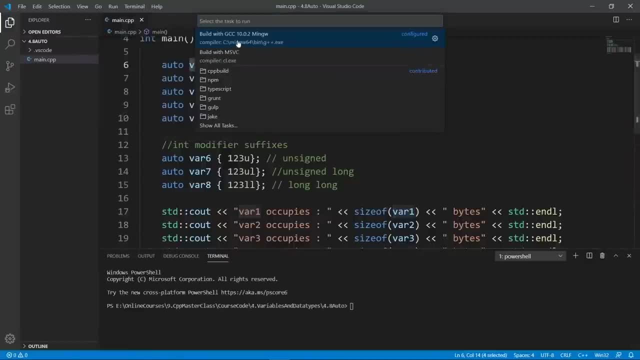 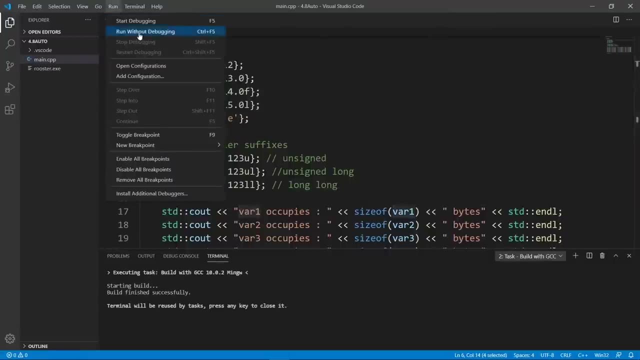 and we're going to go to terminal and run task. we're going to build with gcc and, by the way, if you want, you can build with the compiler from microsoft by coming to terminal here and choose it with world, with msvc, but but gcc is my favorite compiler and i am going to use it if i can. so we're going to hit enter. 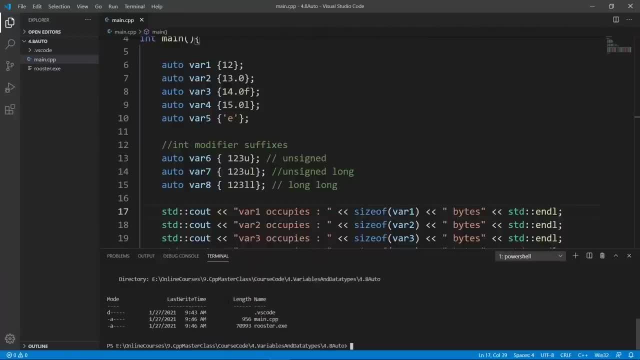 and enter, we're going to see that our roosterexe file is in place. if we run it, we're going to see our sizes. so var 1 occupies 4 bytes in memory. var 2 occupies for 8 bytes in memory because it is double. var 3 occupies 3 bytes because it is a float. var 4 occupies 16 bytes because it is a. 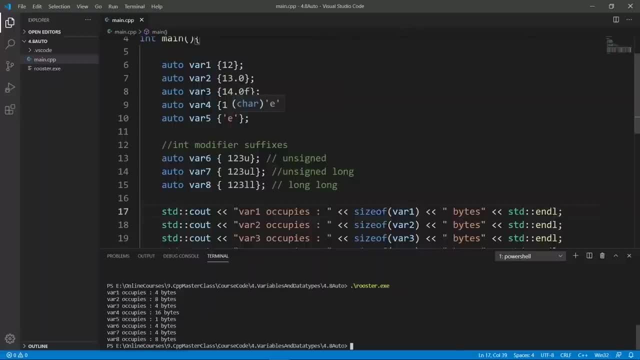 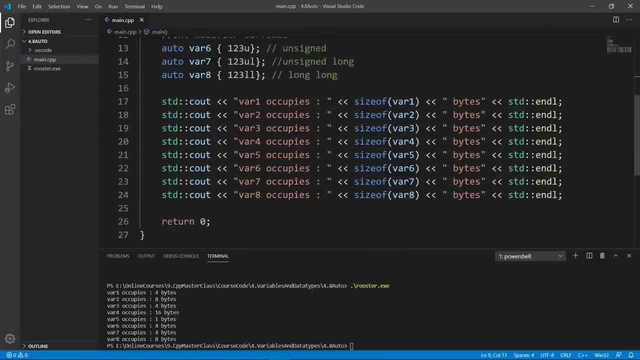 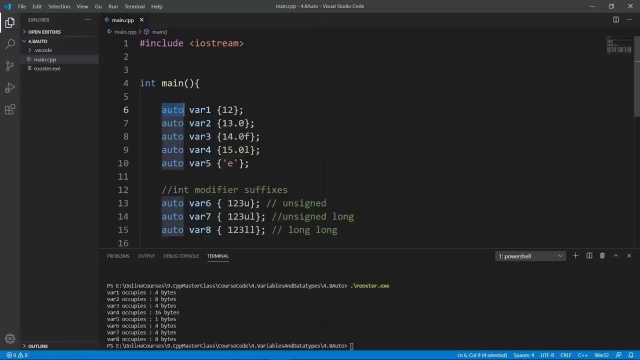 long double and var 5 better occupy one byte because it is a character, and we see the same data for var 6, var 7 and var 8, and this proves that the auto keyword is really doing its job. it is deducing the types for our variables without us explicitly specifying the variable type. 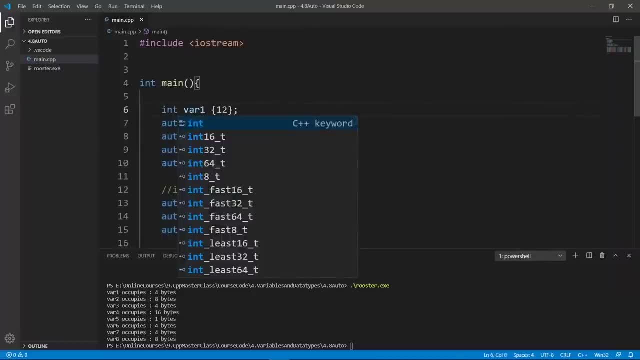 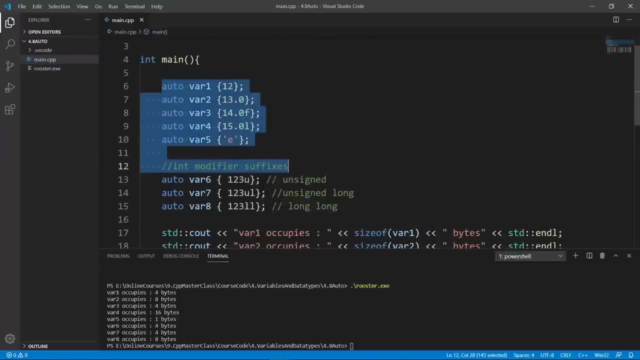 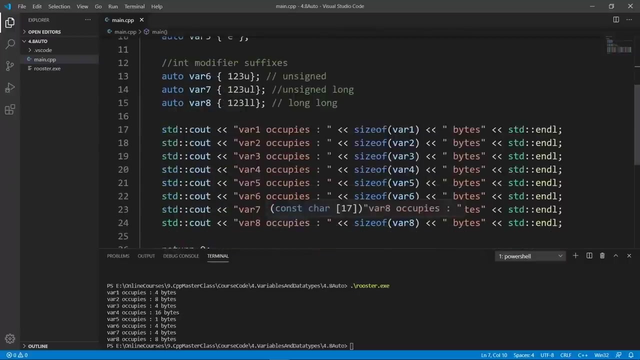 we didn't have to do something like and or double or whatever. we can let the compiler do that for us, and this will come in handy many times. this is really all we set out to do in this lecture, and i hope you found it interesting. in the next one, we're going to look at how we can do assignments. 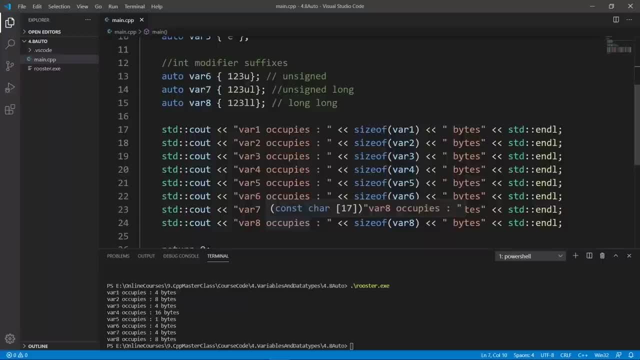 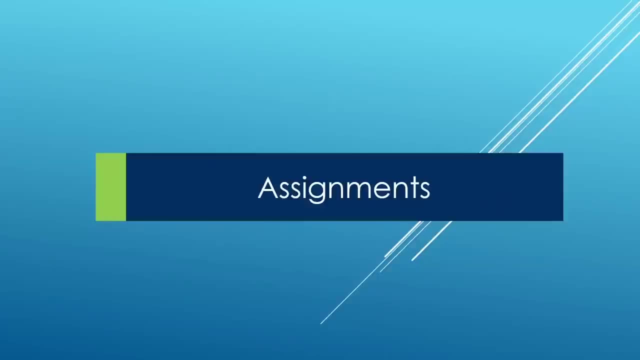 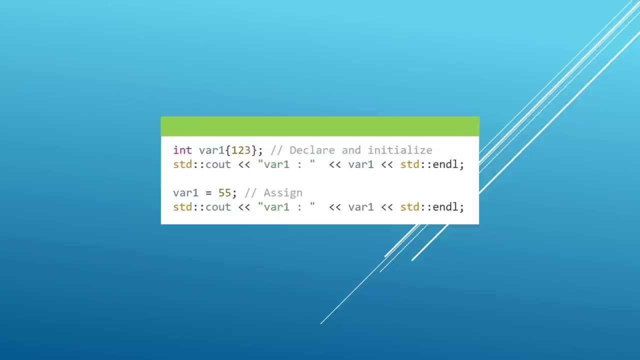 and assign data to our variables in a unified way. go ahead and finish up here and meet me there. in this lecture, we're going to learn about assignments, and the basic idea i've really want to drive home here is that after a variable is initialized- like we've been doing all along- 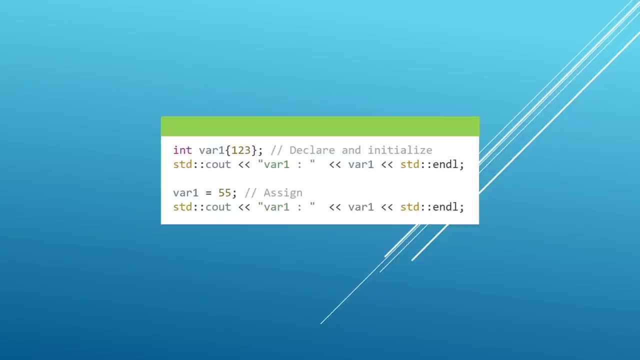 you can later assign a new value to it. for example, here we have var 1 declared. it is an integer, we can print it out and it is going to print 1, 2, 3. but later in the program we can put in another value. for example, here we are putting in a 55 and if we print var 1 it's going to be 55 this time. 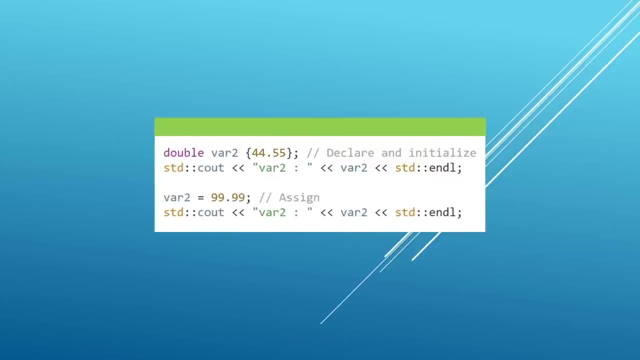 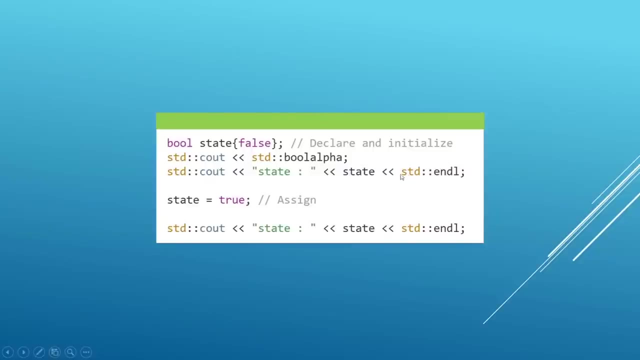 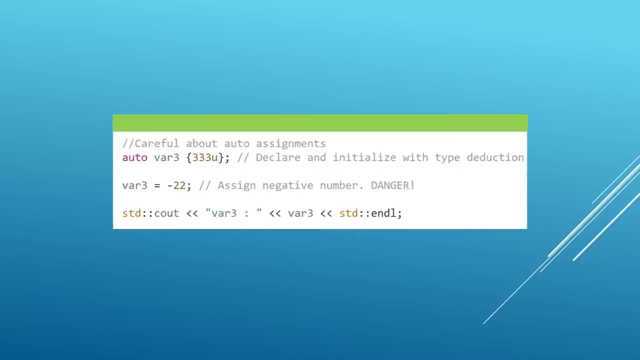 the same idea can be extended to base in the text. we are doing the same thing, boolean. we are doing the same thing. here the state is declared force and we are creating that, and after we are changing this to a true value, and if we print that, it's going to be true. one thing you really need to be careful about is if 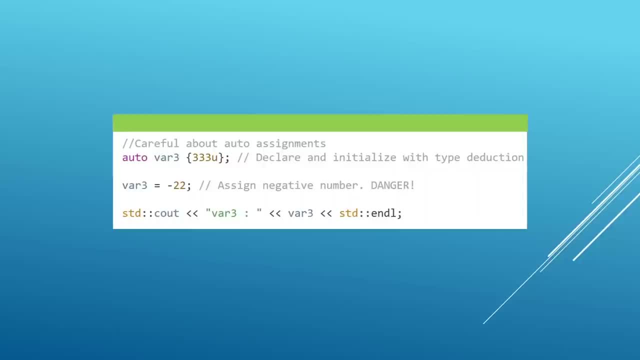 you are doing auto type deduction. the type is not very apparent by looking at the declaration of the variable here, for example here, by looking at auto var three, we don't really know what that is and it is very easy to try and put in a value that is illegal, for example here: 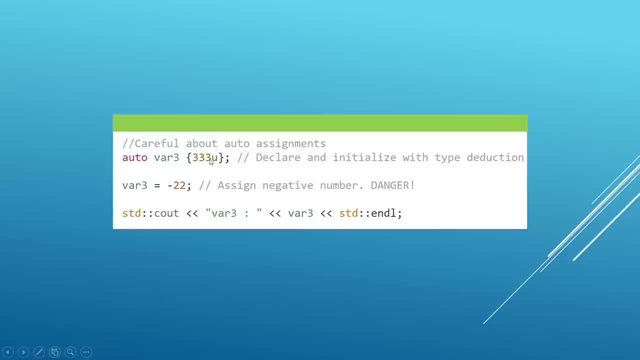 we have deduced an unsigned integer which is only going to store positive numbers, but we are putting in a minus 22 and this is going to be a disaster. we're going to get a compiler error and this is going to be bad. so be careful when you are doing auto type deduction in your assignments that you 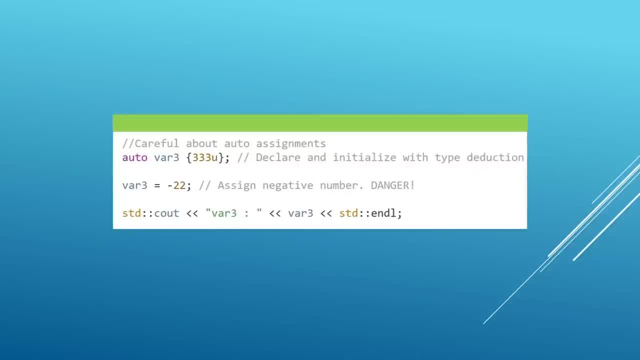 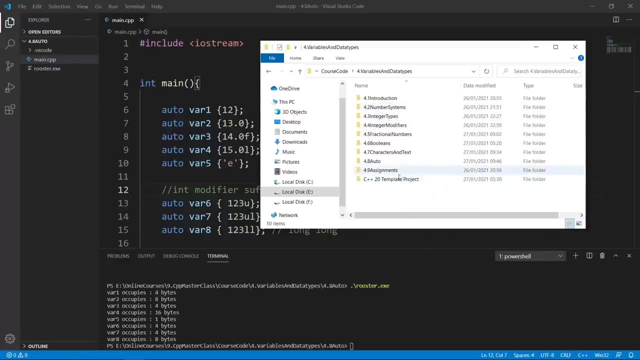 do to your variables. this is really all we have to share in this lecture. let's hop over to visual studio and show you this in action. okay, here i am in my working folder. the project we're going to be working on is 49 here assignments. i am going to grab my template files and put that in this folder. 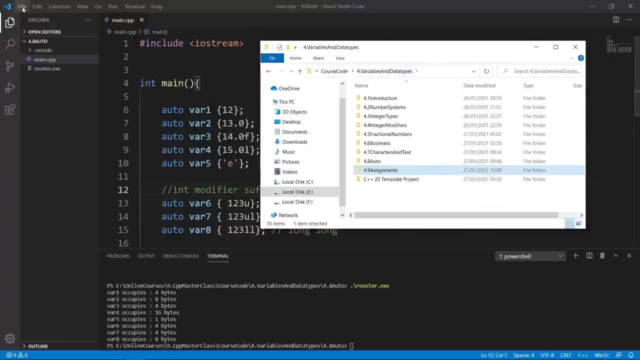 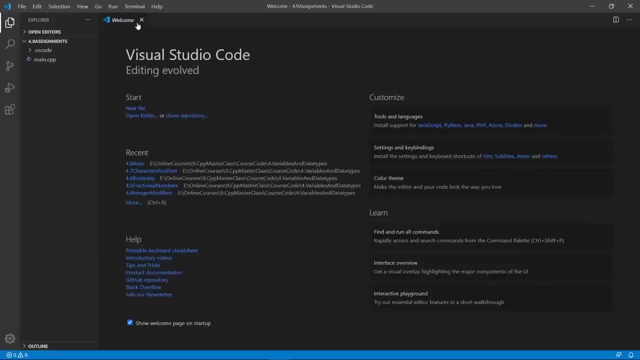 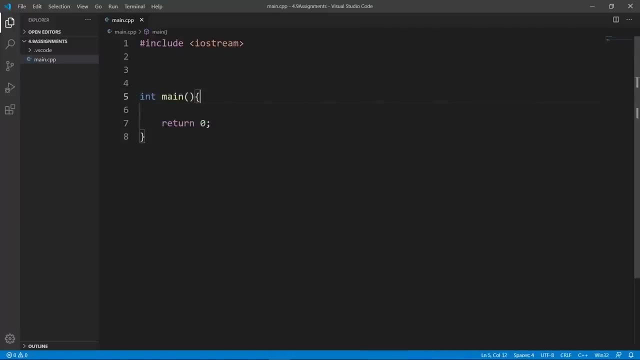 here and i am going to open this up in visual studio code. so let's close whatever it is we have now and open the folder. we're going to close the welcome screen here- we don't want it- and remove whatever we don't want from this file. here, the first thing we want to do is put in the code for our integer variable var1. 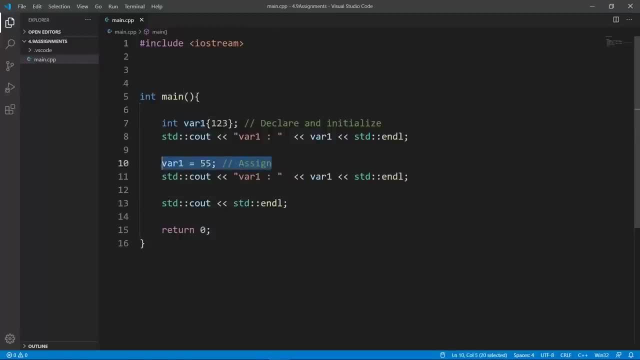 and show you that you can assign a new value to it after it was initialized. and if we run this code, we're going to see var1 to be 1, 2, 3 and the second statement is going to say: var1 equals 55, that's. 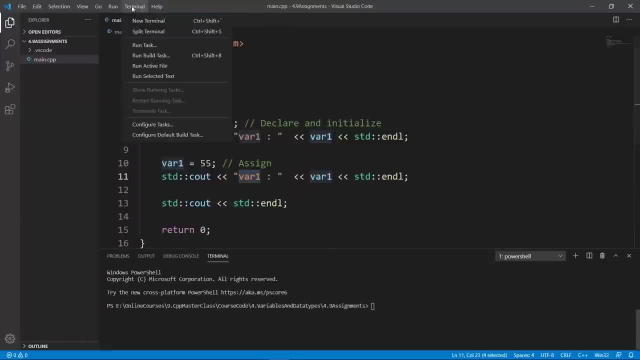 what we're going to see. let's bring up our terminal and we are going to run the task to build with gcc. and if we hop over here in the terminal and do dir, we're going to see that our roosterexe file is in here. if we run it, we're going to see var1 1 to 3, var1 55- exactly what we expect we have. 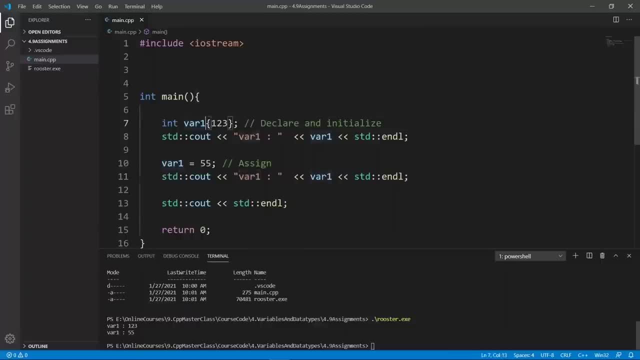 stored in a one, two, three at initialization using braced initialization here. but after, later on in our program we have decided to put a different value in this variable here, essentially reusing it to store something else. this is the basic idea here we can do the same. 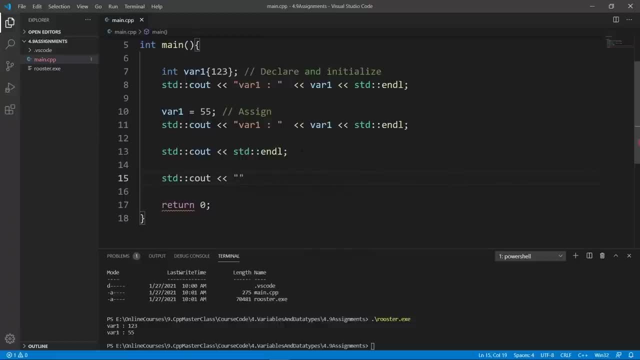 things with doubles. but before we do that, let's put in a separation line so that we can see these things clearly in the terminal, and we're going to go down and put in our code for a double. so we have a double variable called var2. initially it has a variable called var1 and we're going to 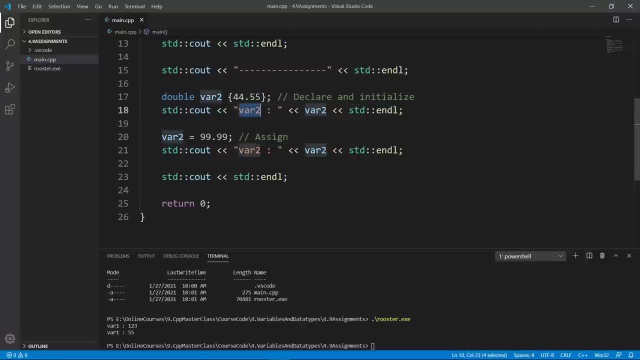 see that it has 44.55 in and then we're going to assign a new value to it and that's going to be 99.99. if we print that out, we're going to see that let's build and see this in action. we're. 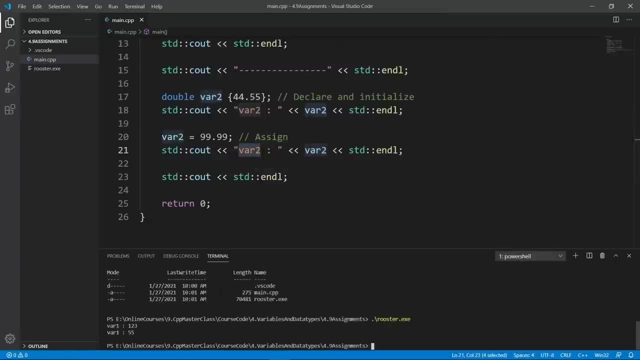 going to build with gcc. if we run the program now it's going to say var1 is one, two, three, var1.55. but we're also going to see that var2 starts out 44.55, but after in the 99.99 it's going to show up here: okay, let's put in another separation line, because we're going. 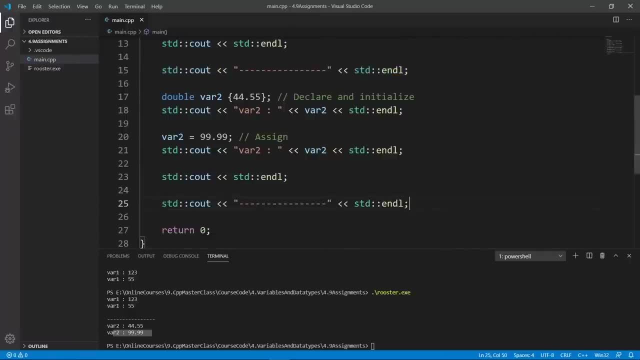 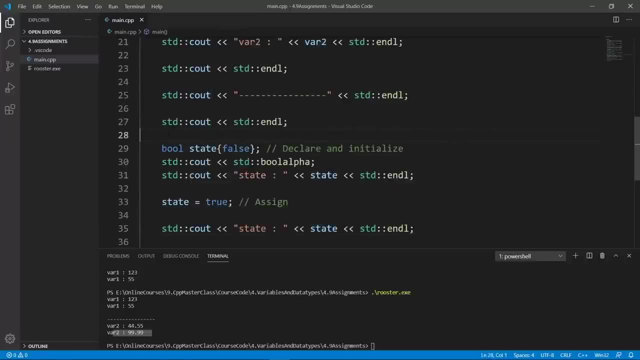 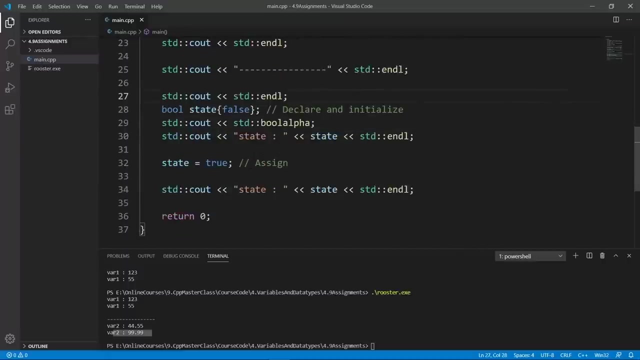 to need that in a minute. we can do the same things with booleans here. we are using this as just an example, but this same concept essentially extends to any other kind of variable you're going to have in your c++ code. if you initialize it with some value, you have the option to change that value. 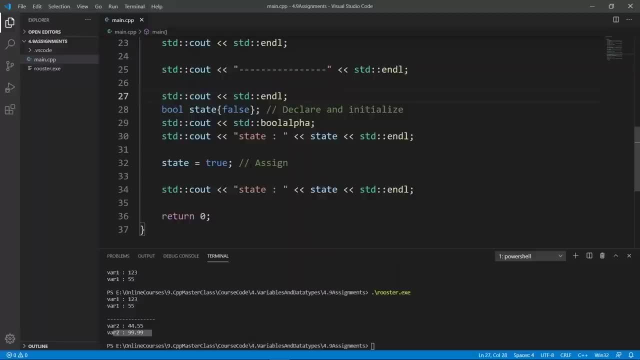 later on in your program by assigning that value to that variable, essentially what we are doing here. the variable state, which is a bool, was initialized to false. we're going to print that out and notice that we have this setting to allow us to see true or false instead of ones and zeros. 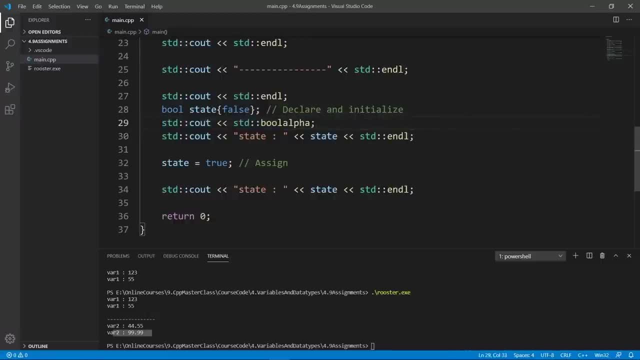 we have seen this in a few lectures back and later on. we are assigning true to this state and we are printing that. so if we print these things out, we're going to see false and true for the state here. so let's build, we're going to use gcc and the world is good if we 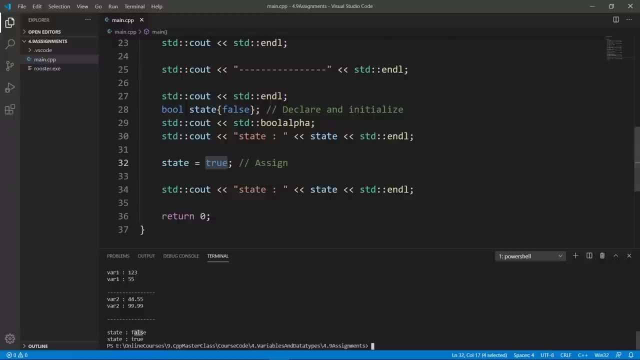 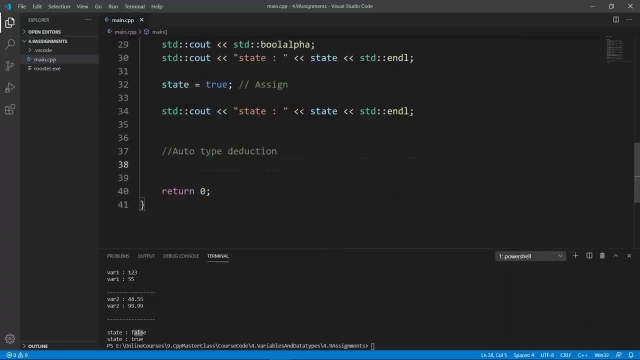 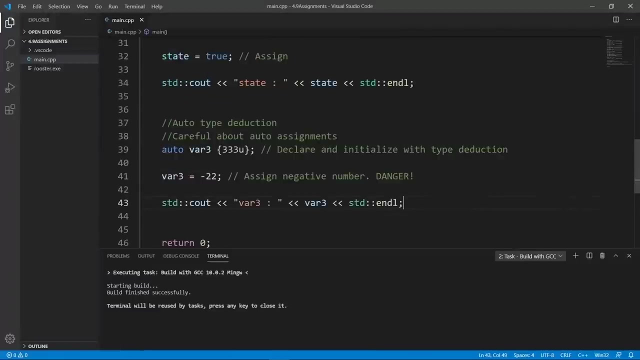 run the program, we're going to see false and true, and it is exactly what we expect again. you really need to be careful when you are using auto type deduction, because you might have some serious problems if you are not paying attention. let's put in the code so that we can play with it. 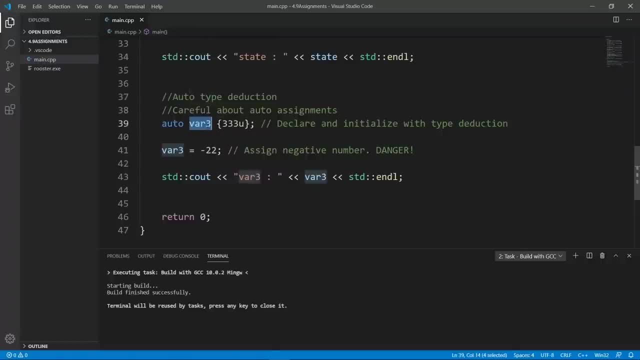 here we have a variable called var3 and the type of it is not specified explicitly. we are letting the compiler deduce this and because our initializer here is an unsigned integer, the compiler is going to deduce that it is an unsigned integer. the problem will come if you try to store in a negative number the compiler. 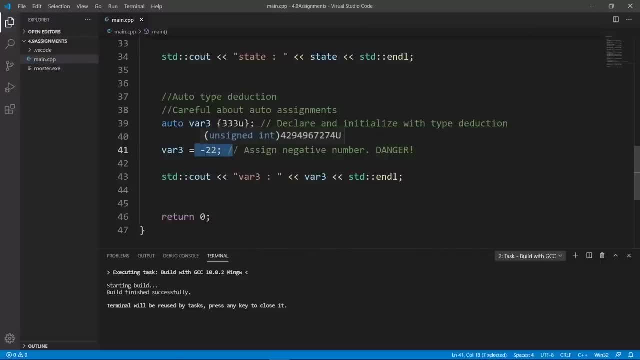 is not going to give you a compiler error. it is going to silently put in some garbage value that we don't really want in there. we want to get rid of it. so we are going to do that. we want a minus 22, and you can see that this is what the compiler is turning our value into. we 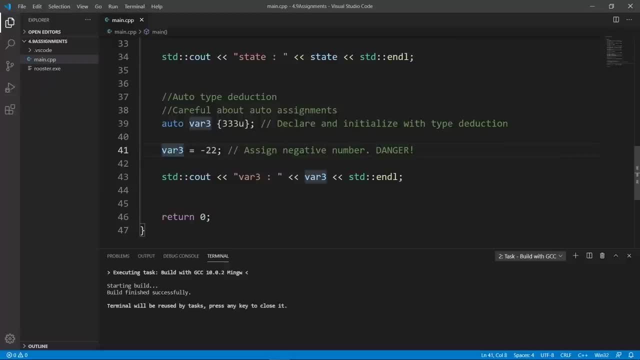 want a minus 22 in this var3, but if you hover over this minus sign here in Visual Studio code, you're going to see that the value that we have in is not what we put in. we put in a minus 22 and we are getting a really large number, close to 4 billion. so this is really something that can go. 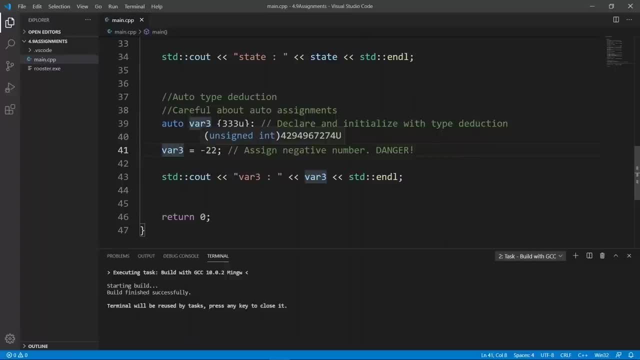 silently wrong in your code and you're going to have a hard time trying to figure out why your code is not doing whatever it is you want. so be careful about this. let's try and build this. so we're going to build with gcc, the world is going to. 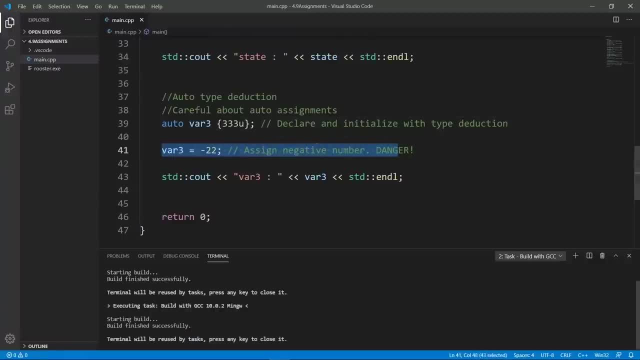 be good. you're going to see that we're not even going to get a compiler arrow if we run this, and we're going to see that var3 is exactly what Visual Studio code guessed. and it is not good. it is this value here and the problem is that the compiler is silently putting in a garbage value and 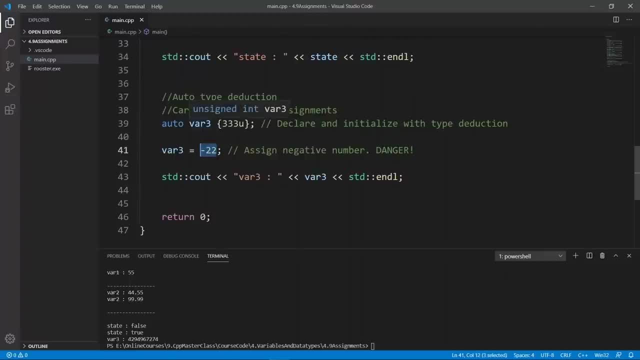 that's not what we want here, because var3 is basically not capable of storing negative numbers, so the compiler is going to do its best and put in a garbage value, and this is not what you want, and you need to be aware of this. this is really all we set out to do in this lecture. I hope. 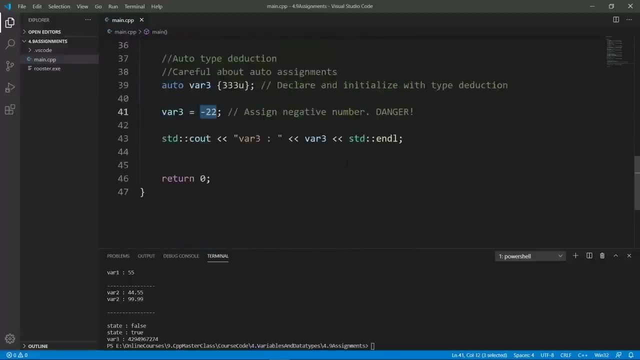 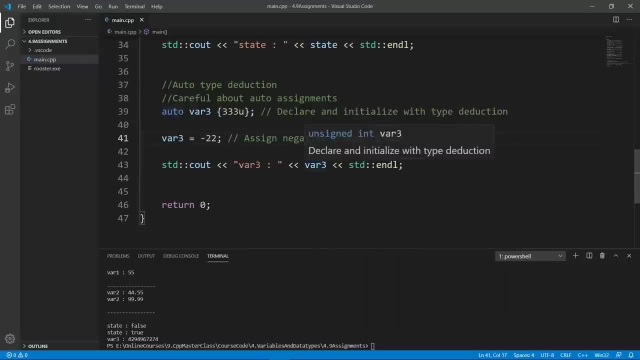 you know about assignments and be careful when you are doing assignments on variables whose types are deduced with auto. and we're going to stop here in this lecture. in the next one we're going to try so in this chapter, go ahead and finish up here and meet me there. in this lecture we're going to recap. 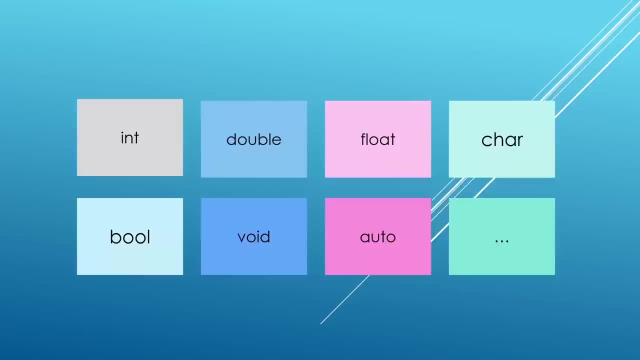 what we saw in this chapter- and this chapter was really all about variables and data types. we had a chance to look at different types that we can use in C++. we saw that we have fundamental types we can use to represent integers, floating points, booleans, and we also saw that we can do type 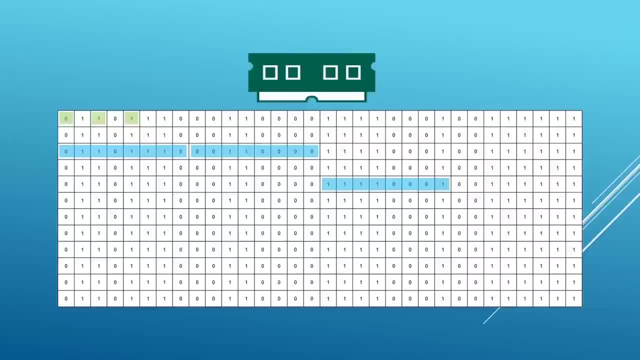 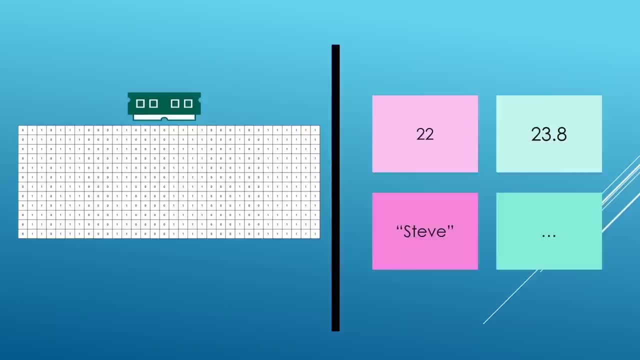 deduction with auto. we had a chance to make it clear that data is represented in memory as zeros and ones and that there are some kinds of transformations we do on these pieces of data to turn them into a form that is easily usable and manipulable by humans, and we saw that for integral types or integers we could. 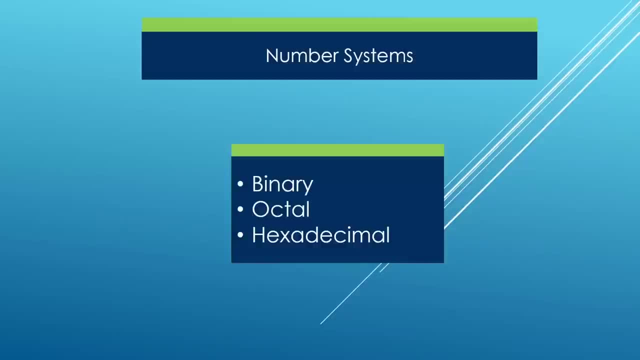 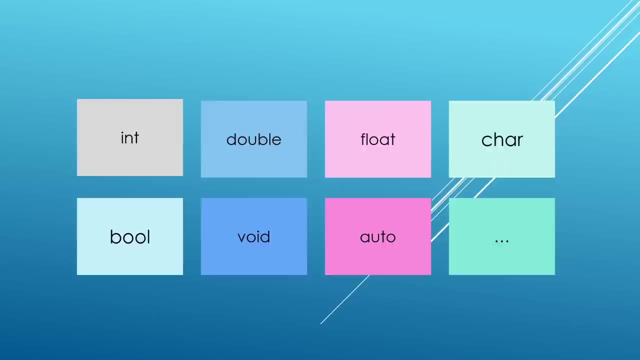 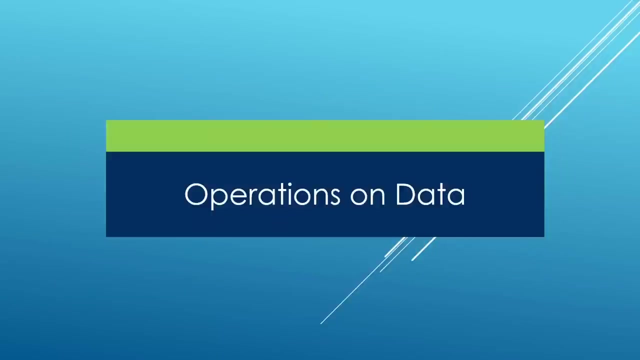 do that through number systems and we had a chance to look at a few number systems like binary, octal and hexadecimal, and we had a chance to play with all these variable types in Visual Studio code and see the nuances of how you really work with them. I would like to welcome you in this new chapter and this one we're going to be. 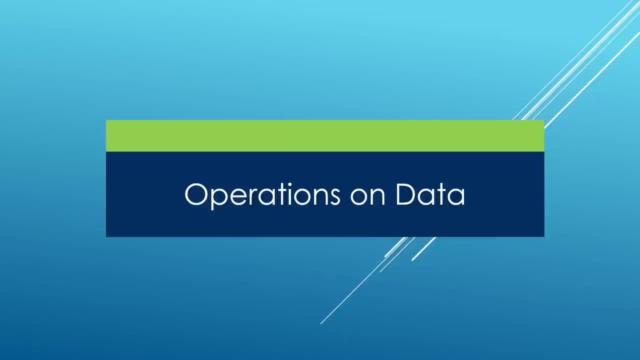 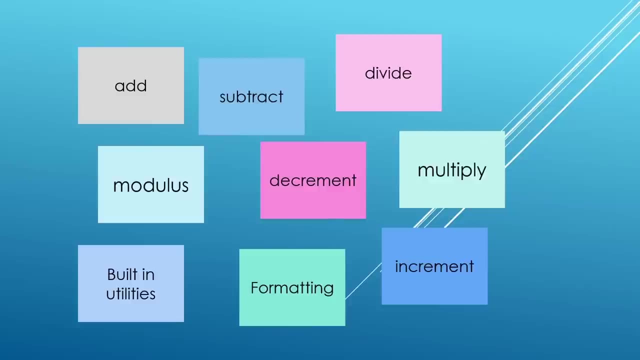 looking at operations we can do on our data, and there is a bunch of them. we can add things up, we can subtract numbers, we can divide numbers. we're going to see all kinds of crazy operations we can do on the data, all the variables that we have in. 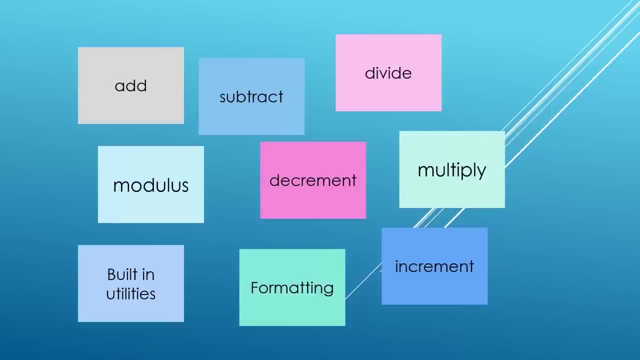 our C++ program. we are also going to have a chance to look at how we can format stuff when we print them out, to stdc out, and we are going to be using some utilities from the C++ standard library to do some operations on our variables. this is going to be a fun chapter. I can't wait. 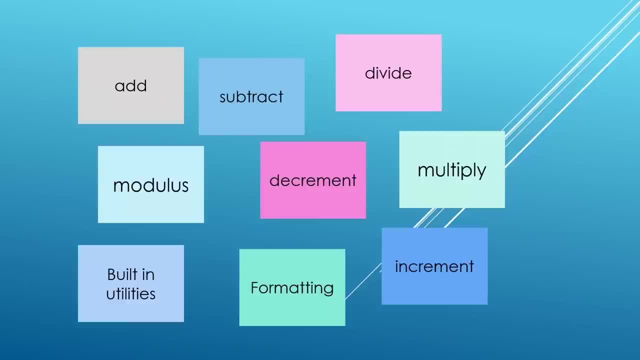 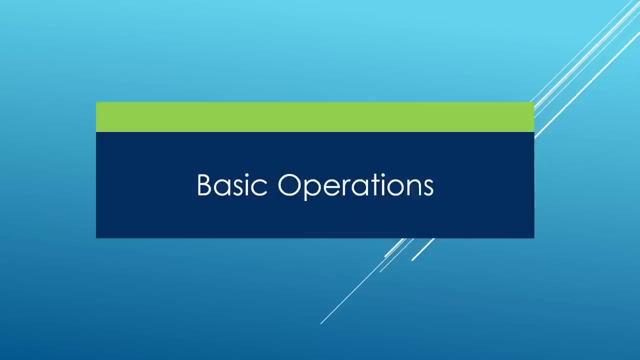 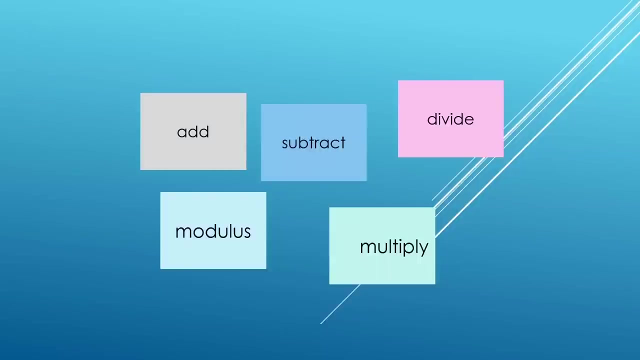 to get started, let's go in the next lecture and start doing this. in this lecture we're going to be looking at some basic operations you can do on the data in your C++ program and we are going to be specifically looking at addition, subtraction, dividing numbers, the modulus operator and multiplying stuff. we have seen addition before. 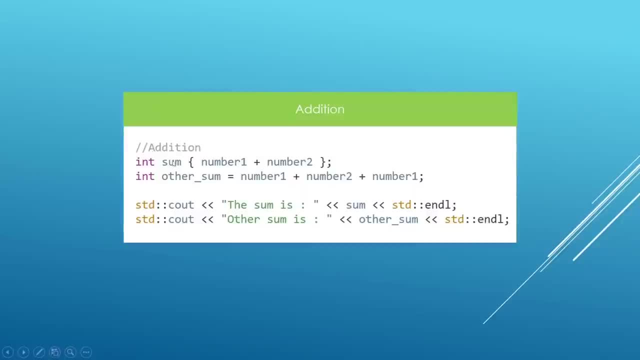 here we have a simple example. we have a variable called sum and we are initializing it with two numbers that we are adding up, number one and number two. this is something you can do in your C++ program. you can also do some other things. for example, we have 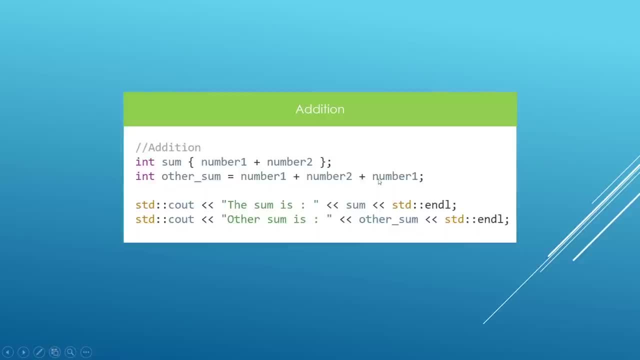 another one called other sum, and we are adding up some other numbers and we are going to collect the result into this other sum variable and we're going to print these things out so that you can see them on your command prompt. this is how you can do addition and we're going to have a chance. 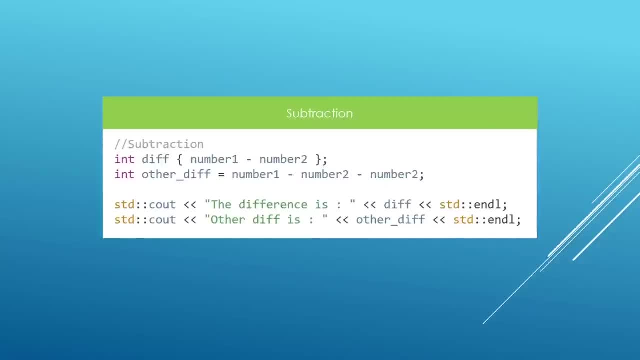 to play with this in Visual Studio code in a minute. we can also do subtraction, we can take a number and do minus another number, like we are doing here. we're going to store the results in this div variable and we can do some other things, and down here you see another example in. 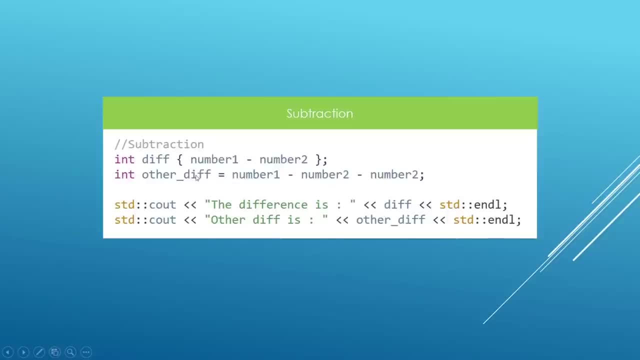 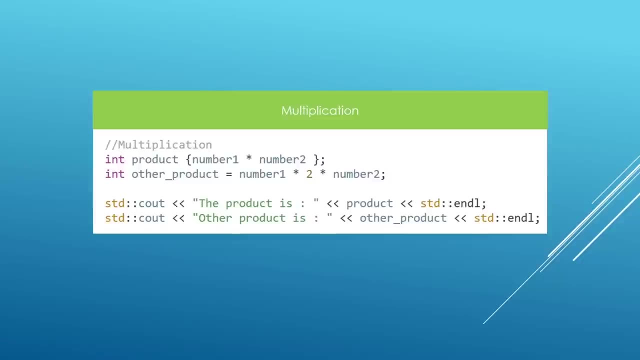 other div. here we're going to subtract numbers and store the result in other def, and we are also going to print this out. you can also multiply stuff. this is how you can do this. you use this operator here. it is the star operator, and this is an operator that many programming languages use to do. 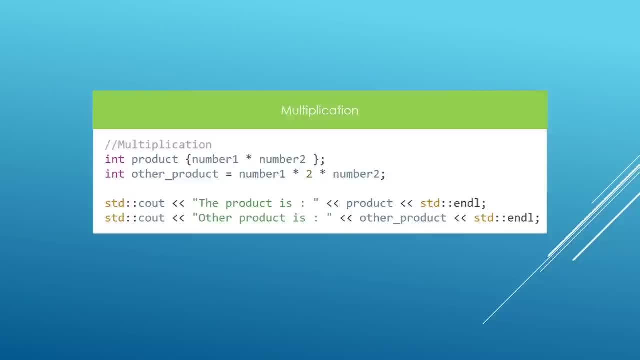 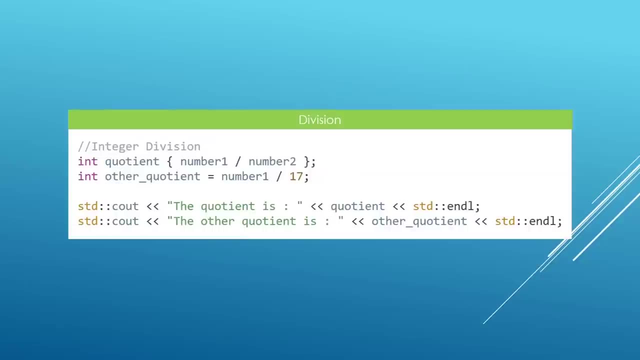 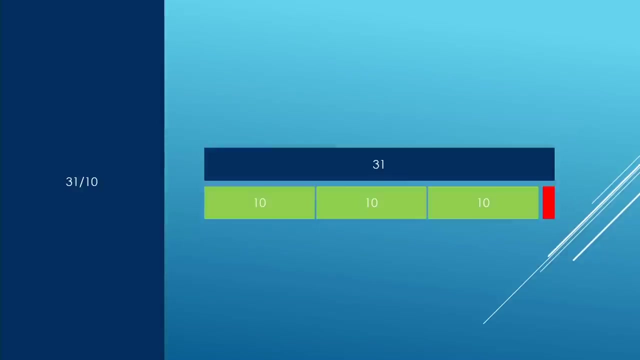 multiplication. you should get familiar with this and again, we print out the result so that you can see that this is actually working. we can also do division. division for integers is a little tricky. if you are seeing this for the first time, if we take, for example, 31 and divide that by 10, we're not going to get fractional numbers. C++ is going. 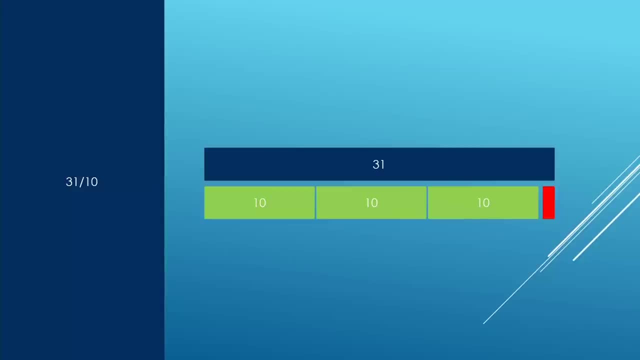 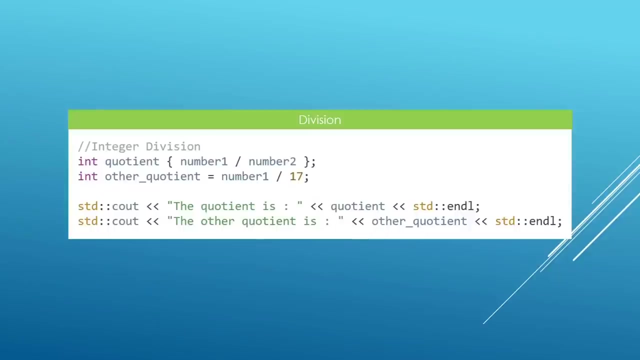 to try and figure out how many times it can fit 10 in 31, and we are visualizing this here. so in 31 we can only fit 10 three times. so the result of 31 is going to be three. this is the meaning here. okay, with integer division you're not going to be getting fractional numbers. this. 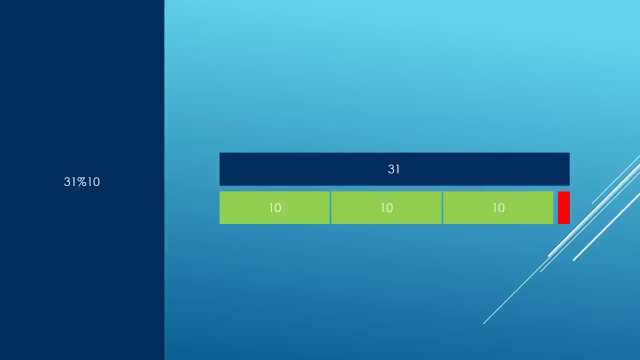 is something you should really understand. we have another operator that is called modulus operator, and this operator is represented by this percentage symbol that we are doing here, and the result of this operation here is going to be what remains after you have done the division of 31 and 10.. and here the result is going to be one, and you might be. 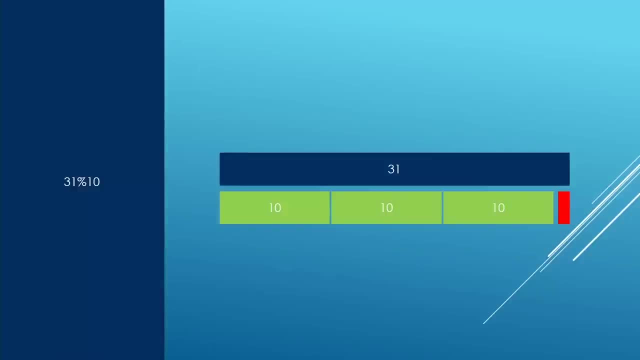 wondering why this is useful. it is going to be useful in many applications and I think we're going to have a chance to play with this later in the course, but right now, you just need to be aware of this operation and what it does. okay, these are the operation we're going to be learning about, and 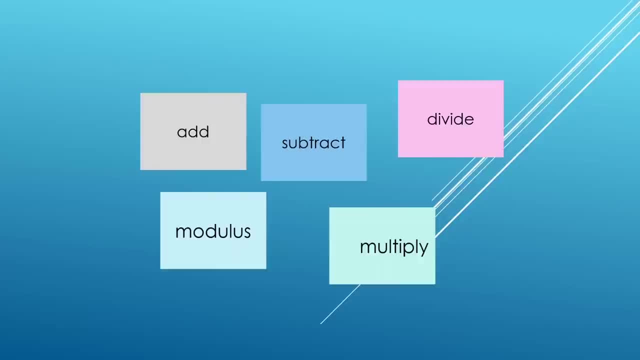 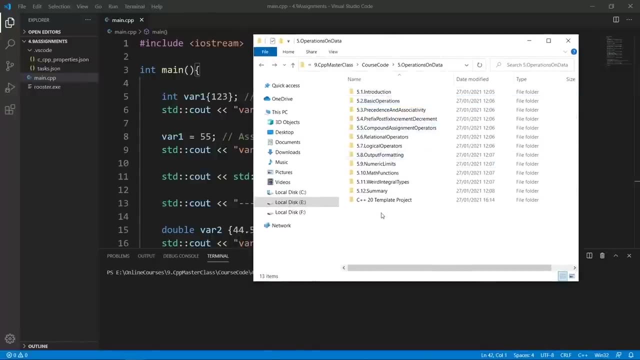 playing with in this lecture. let's head to Visual Studio code and actually play with this. okay, here we are in our working folder for this chapter. you see that I have prepared all the lectures we're going to do in this chapter and I have my c++ 20 template project in place. I am going to do what 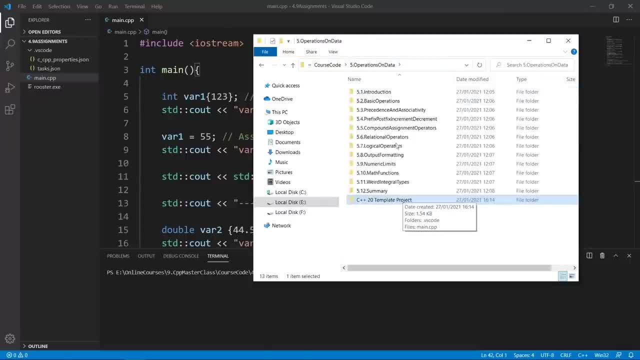 we have been doing all along. so I am going to take these files and put them in the current lecture, which is basic operations, and I am going to paste those in and I am going to open this folder in Visual Studio code. so let's do that pretty quick. we are going. 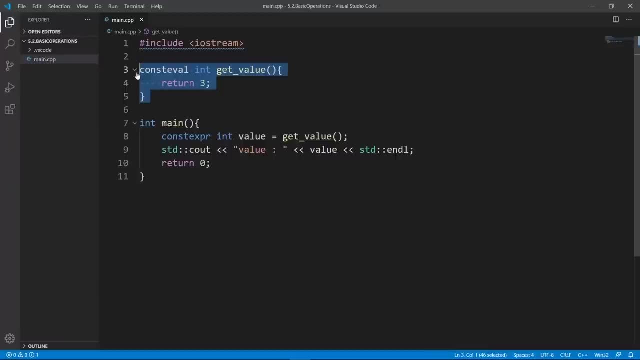 to close the welcome screen here and we're going to open our main cpp file and we're going to remove things we don't need here. the first thing we want to play with is addition. so we're going to say that and we're going to declare two into variables. we're going to call this number one and we're. 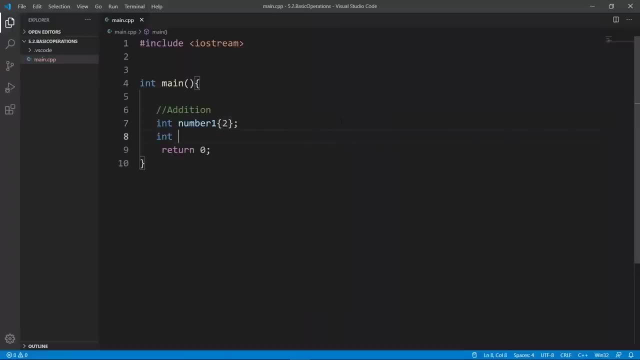 going to put in a two, for example, and we're going to do a number two and we're going to put in one plus number two and we're going to store the result of this operation and the result variable here. so what we can do is say stdcl and we're going to print the result we can try and compile. 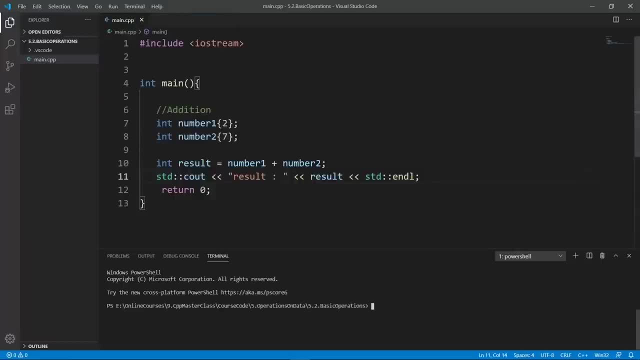 this and see the result. let's open our terminal here and we're going to build with gcc as we always do. the build is going to go through and if we run rooster here, we're going to see that the result of our operation is nine. so this is how you can do addition. you can also do subtraction. 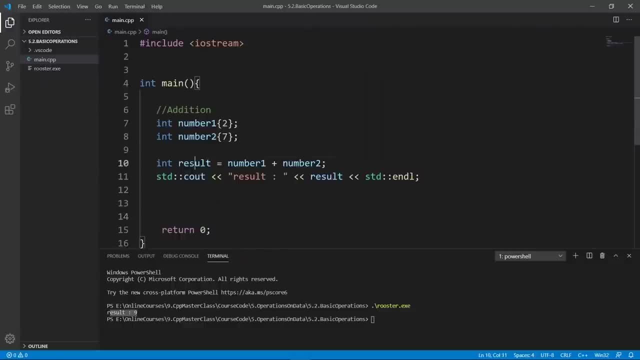 and here we know to declare a new variable. we're going to store the result in our result variable here. so what we're going to do here is say subtraction and we're going to say result equals. for example, let's take number two minus number one. this is the operation we want to do. 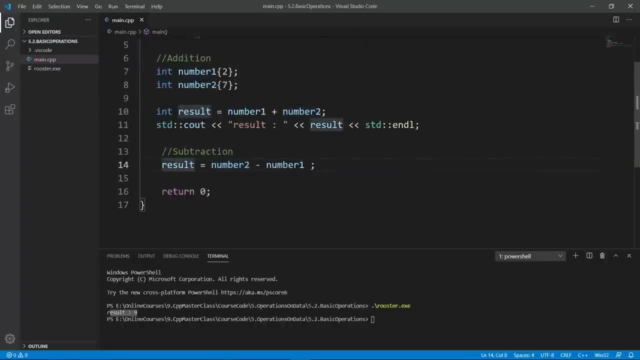 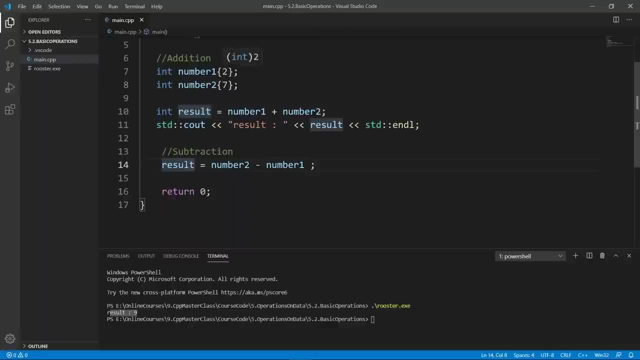 result here is going to be a five because we are taking seven and subtracting two. i hope this makes sense. so if we grab this line here and paste it in here so that we save on some typing time and try to build it m, we're going to run the world task with gcc and we're going to run rooster again. 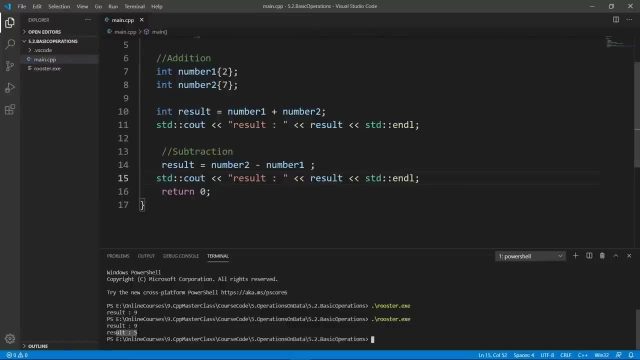 it is going to say: result is five because we are taking seven from basically this program. we are and minus two. here the result is going to be five. we can also do a subtraction operation that is going to result in a negative number. so for example, we can say: result equals number one minus. 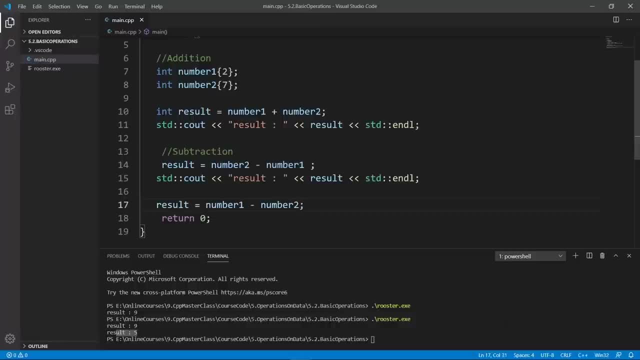 number two and this is going to give us a negative number, because two minus seven is going to be minus five. so we're going to print that here. i'm going to paste the same because i still have this on my clipboard: if i build with gcc and run my program, we're going to get minus 5 as a result. 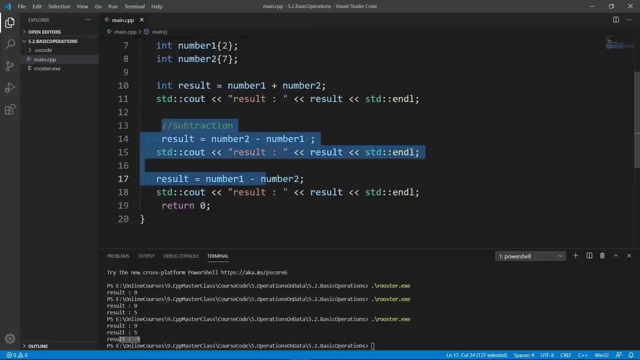 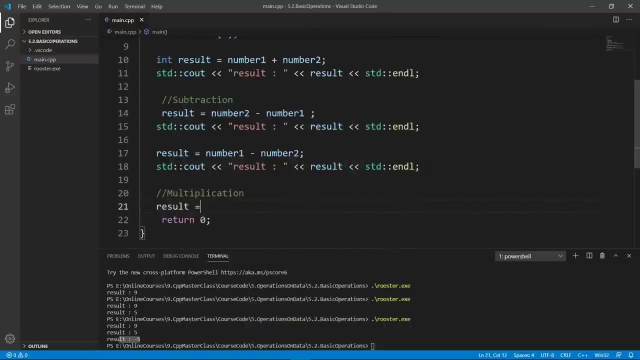 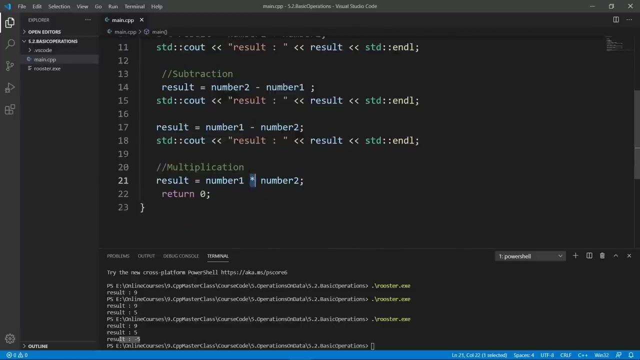 of this operation here. this is how you can do subtraction. we can also do multiplication. so let's go down here and say that, and we're going to say: result equals number one multiplied by number two, and this is the operator we use to do multiplication in programming languages. we're 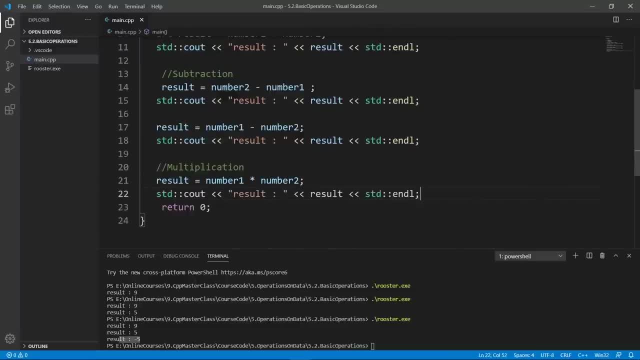 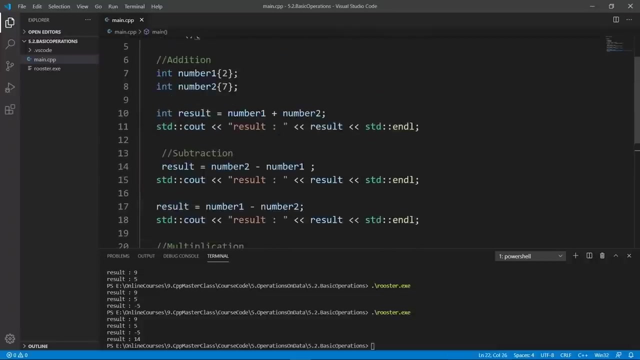 going to put in our print statement here and we're going to world with gcc and if we run rooster now, we're going to get 14, because we are taking 2 and multiplying that with 7.. this is how you can do multiplication. so what happens if you? 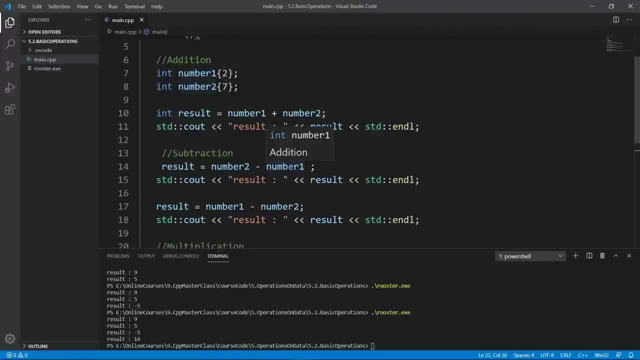 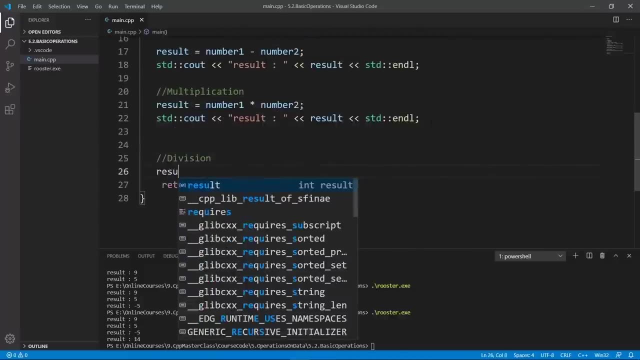 take 7 and divide that with 2.. try to give this a guess based on what we saw in the slides. we're going to go down here and do division and we're going to say result equals number two divided by number two, and we're going to say result equals number two divided by number two. 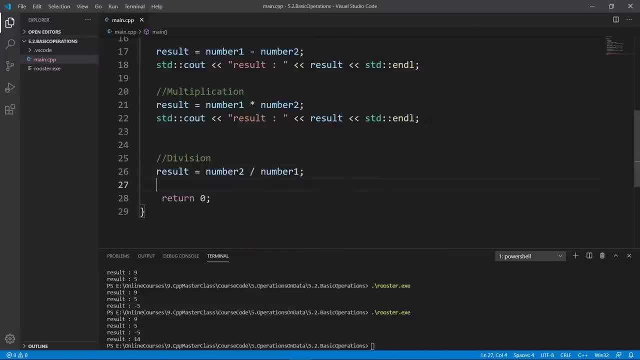 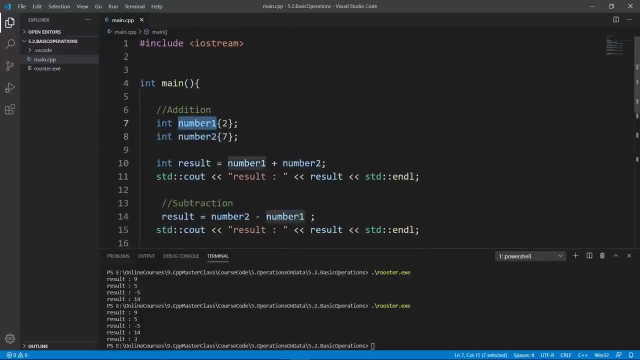 divided by number one and uh, we're going to try and print this out. if we build this, the world is going to go through, and if we run this, we're going to see that result is three mm-hmm. so to really make sense of this, let's look at these numbers. we are taking number two and dividing that with. 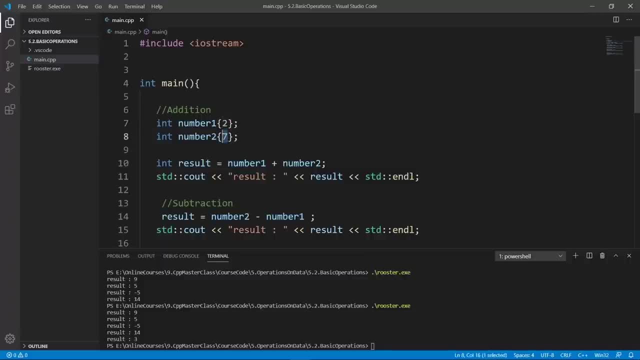 number one. so it is seven divided by two, and because we can't store fractional numbers in a integer, the fractional part is going to be basically chopped off, and we're going to do this. we're going to store a three, because two can fit in seven only three times. i really hope this makes. 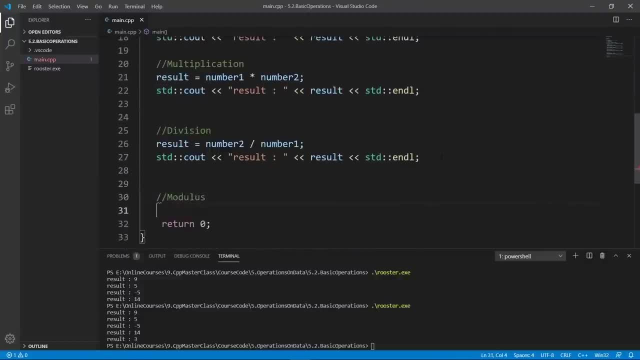 sense, the last operation we're going to look at is modulus, and it is a way to capture the reminder of a division operation. so we're going to do result to play with us, and we're going to say number two, and we're going to say modulus, using the percentage operator here, and we're going to 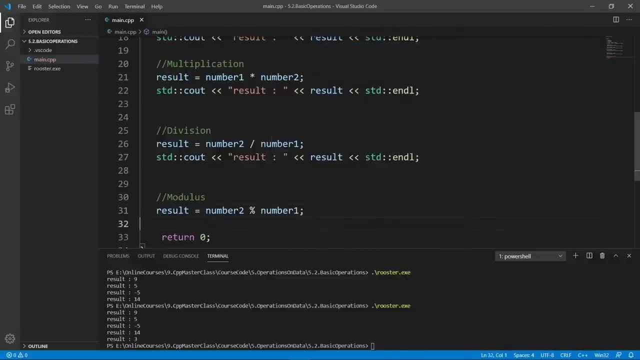 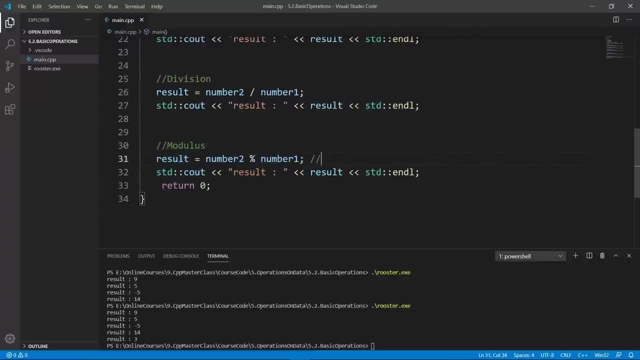 say number one, and we're going to print the result, and we're going to say number two and we're going to say the result of this and, uh, take a look at this here and try to guess what we're going to be doing. what we're doing here is really seven modulus two, and we're going to stake seven. 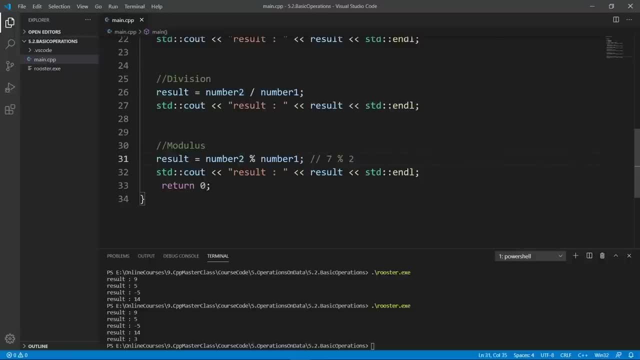 divide this by two and the reminder of that is going to be one, and that's what we're going to store in this result variable here, and if we print that, we expect to get a one here. this is what modulus does. let's build. and, uh, with gcc, the world is going to go through. if we run rooster here, we're going to get a one. let's do. 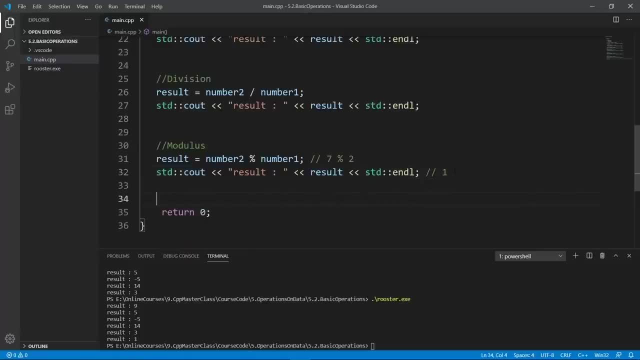 what we used in the slides so that this really makes sense. we're going to go down here and do: equals 31 modulus 10.. this is what we used in the slides, so we're going to print the result here and here we are really asking what is going to be the reminder if we take 31 and divide that by 10. 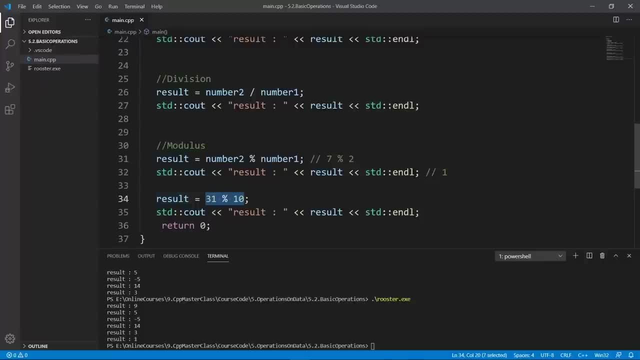 and that reminder is going to be going to be the number of times 10 can be stored in this result variable. so here we're also going to get a one. so let's weld with gcc and we're going to run the program and we are also going. 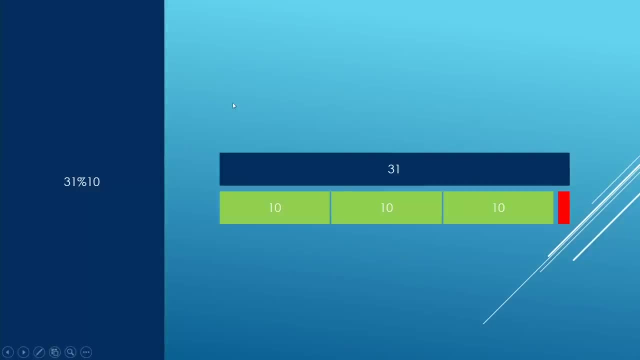 to get a one down here again. the modulus operator can be hard to understand for beginners, but it is really capturing the reminder of the division. again we can see that here we are asking: how many times can tan fit in 31.. and we visualize this here: it can only fit in 31. and so we can see this is how many times 10 fits in 31. and we visualize this here: it can only fit in 31.. 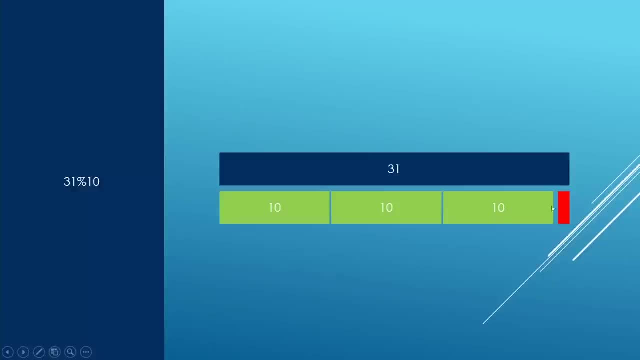 fit in three times and the reminder is going to be this red thing. you see, here it's going to be one, and when we do a modulus operation here, we are interested in that reminder and that's what we're going to be storing in whatever variable that is capturing the result of this modulus operation. 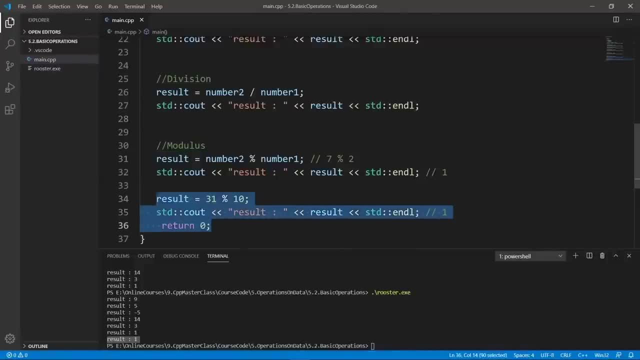 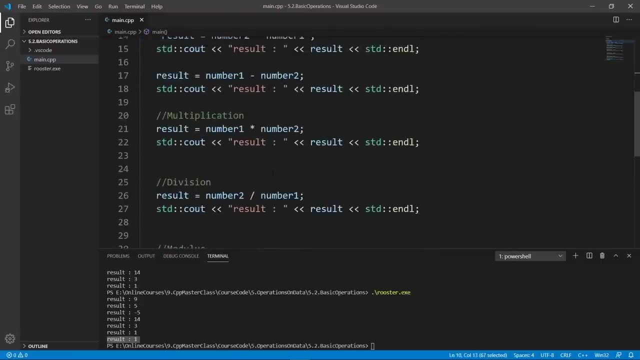 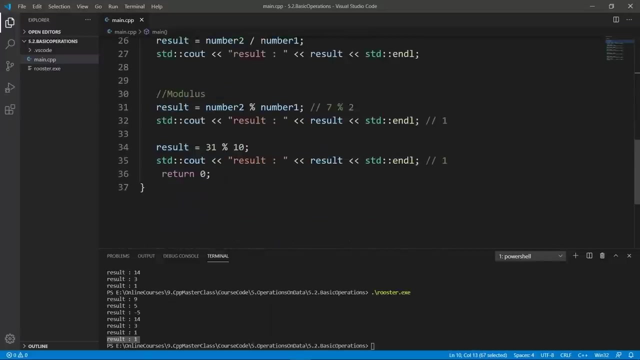 and that's what we basically have here, and this is really all we set out to do in this lecture. now i hope you have a good understanding of these operations you can do on integers- we have used integers here- but you can really do these operations on numbers, except for the modulus. 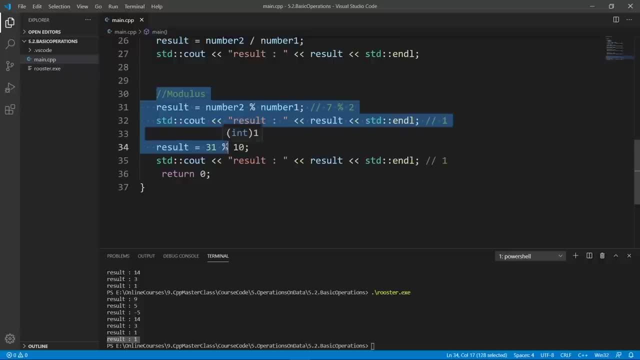 operator which is really going to make sense for integral types. so you can't really do modulus on floating points or fractional numbers. that's not going to make any sense at all. we're going to stop here in this lecture. in the next one we're going to learn about. 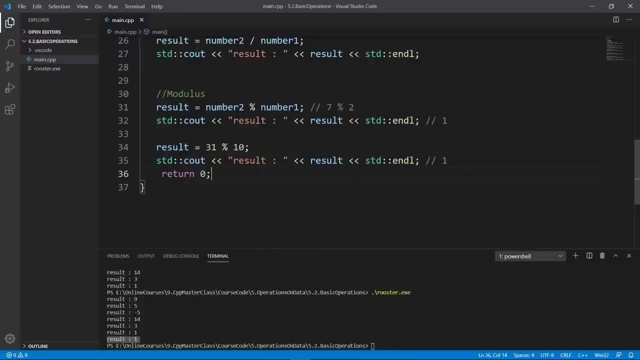 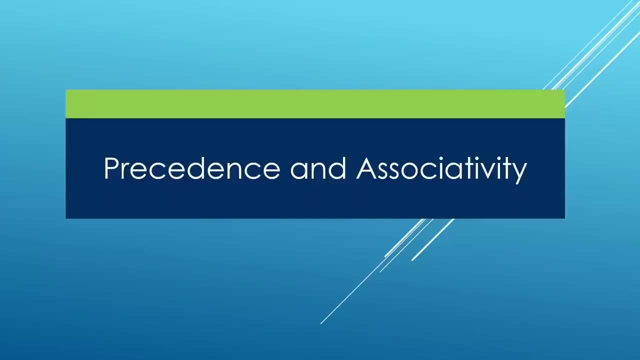 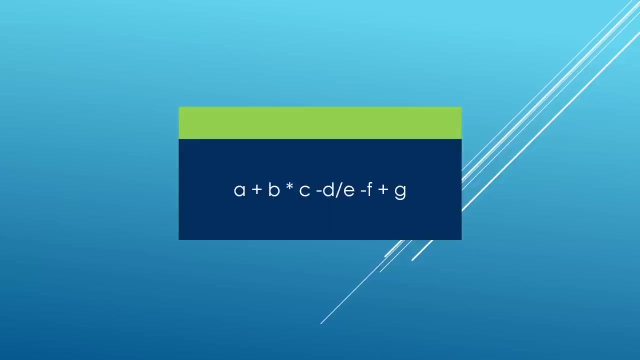 precedence and associativity, a very important concepts for your operations in your c plus plus programs. in this lecture, we're going to learn about precedence and associativity. so what do we mean by precedence and associativity? really, what we mean by this is a set of rules that we can 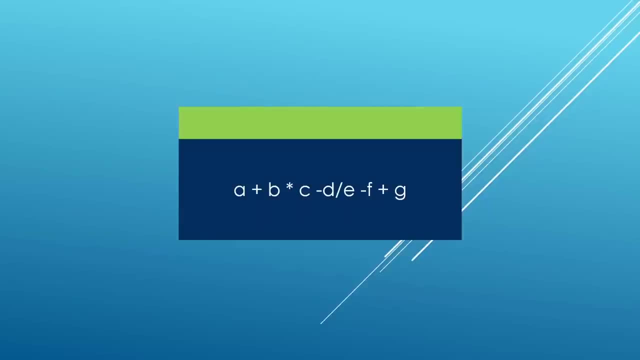 follow to know what to do when we have multiple operators in the same expression, like in the example we have here. if they tell you to evaluate the result of this expression, if we don't have clear rules to follow, we might have multiple answers. we want to know which one is right or wrong. for example, one might want to 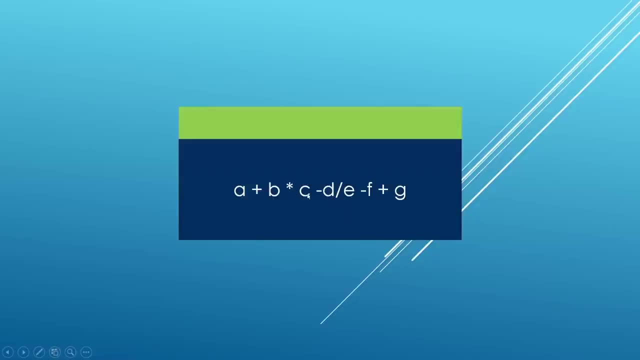 do a and b first and then do c and then do d. but one might want to do e minus f and do b multiplied by c and then do things in different ways and get different results. hopefully you are seeing that this may be a big problem. what we get from precedence and 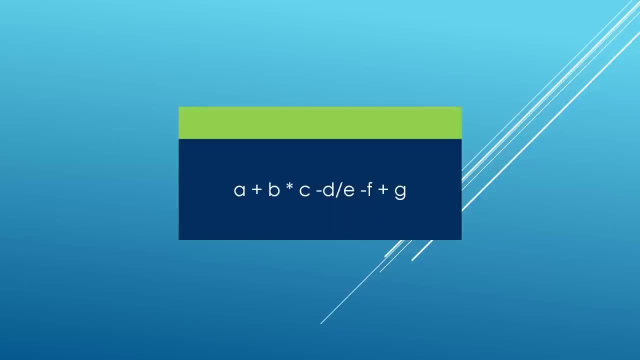 associativity is the rules we can follow to know which operator we have to do first. for example, in c plus plus, the multiplication and division operator have to be done before you do addition and subtraction. and if you want to evaluate this expression here, you're going to have to do b and c first and then do d and e once you have those. 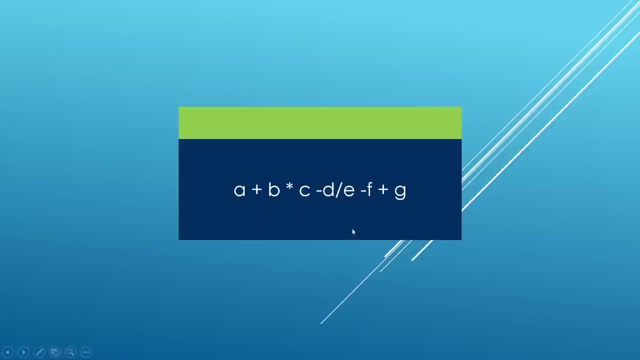 results. then you can do addition and subtraction. but the question remains still: what do we do first if we have only addition and subtraction in an expression and we solve that problem with associativity. associativity defines if you do the operations from the left or from the right. 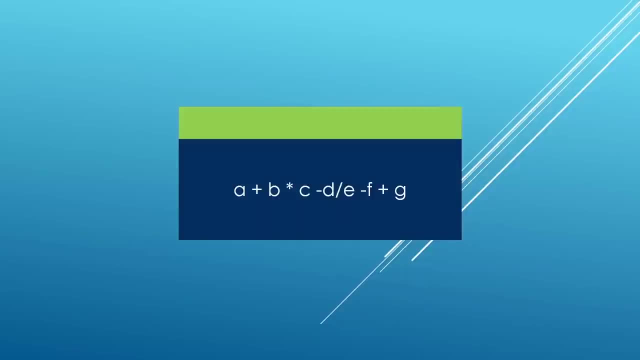 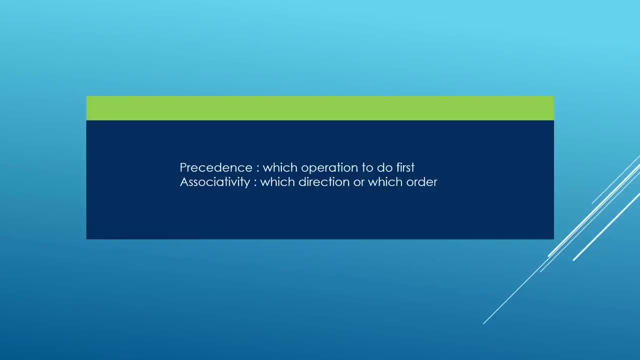 and again, these things might not make sense. yet we're going to do an example and you're going to really see what is meant by this. to summarize: precedence tells you which operation you can do first, and associativity is going to tell you in which dock we want to do the operation. you can do the operation from the left, and again this thing might not make sense yet. we're going to think about how to solve it first. but you have to have and e and c will come up, and Ми, t, me, a, and and a numeric way you can base them. in my opinion- you might want to check them- amount and size something. 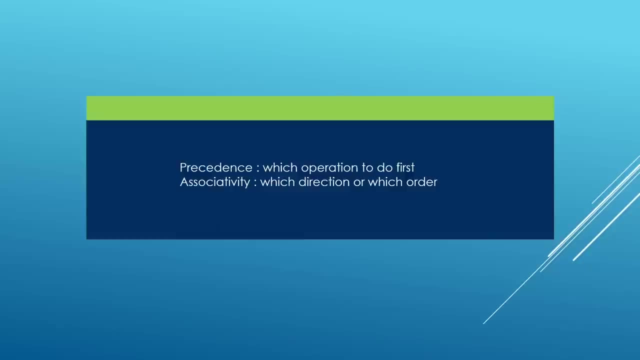 them and put them in place- a stage one difference. but the common question has to be based on what's you, in which direction you're going to go, from the left or from the right? and some operators are going to be left associative, and that means that you're going to start evaluating them from the 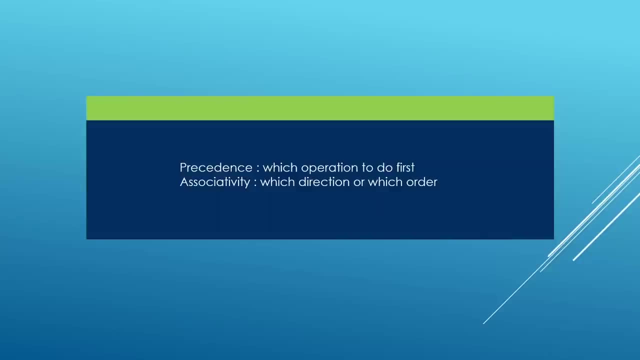 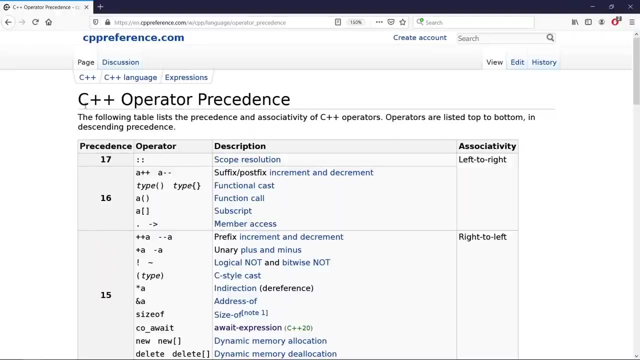 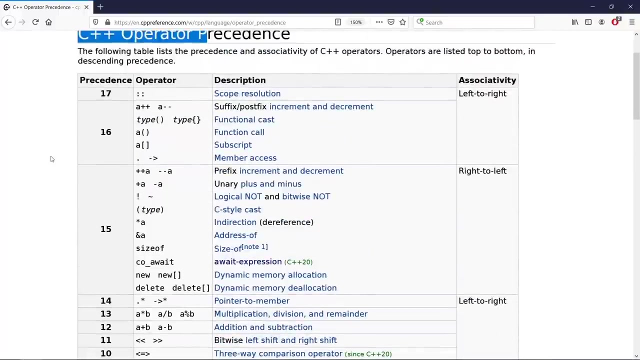 left. some operations are going to be right, associative, and you're going to start evaluating them from the right and i am not making these things up. there is actually a c plus plus operator precedence table that you can consult to know which operators you should do first, if you really 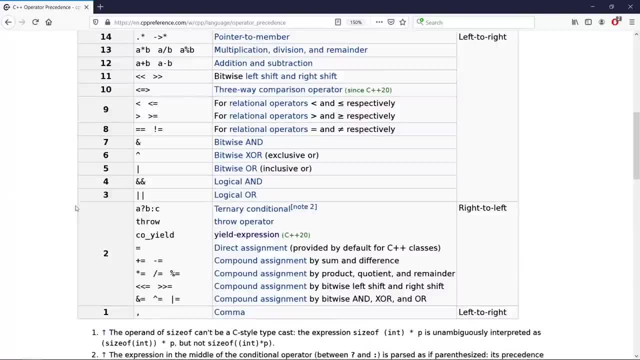 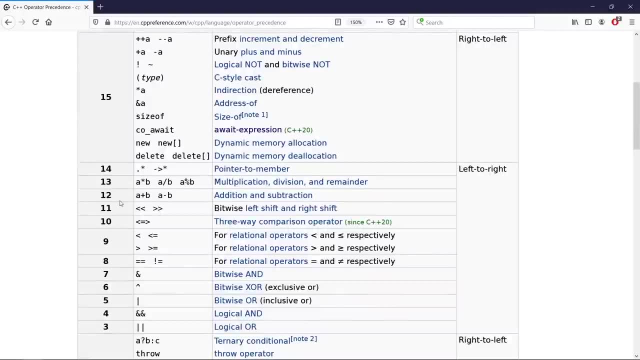 are evaluating this thing with your mind okay. for example, if you look in this table, there are many operators we haven't seen yet, but that's not the problem. the most important thing here is to know what precedence and associativity are and when we get to learn about these new operators. 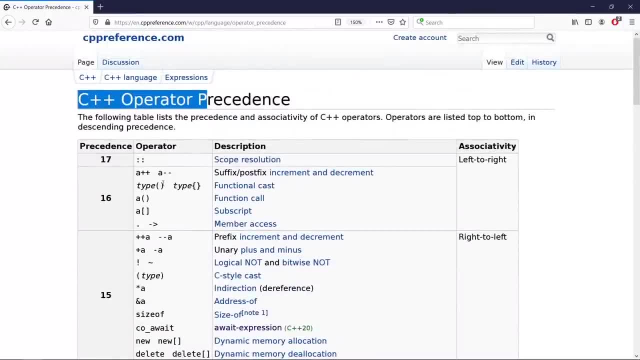 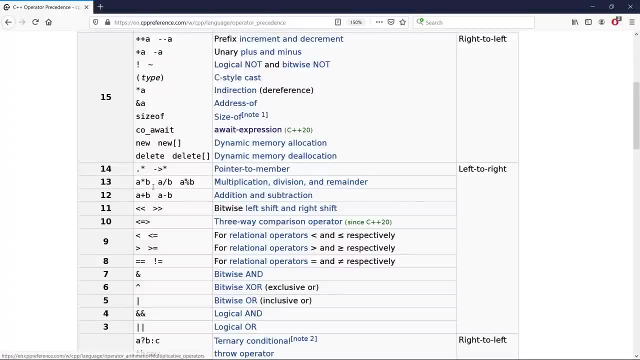 you can come here and know where they sit. in this precedence table, for example, we know how to do addition, multiplication and modulus. we see that the precedence for multiplication, division and modulus is higher than for addition and subtraction and we can use this in our operators to know which one is going to be. 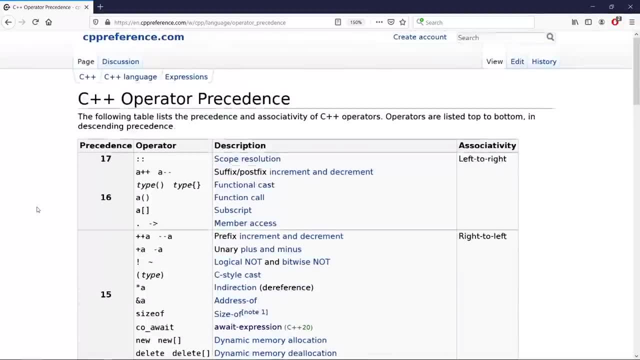 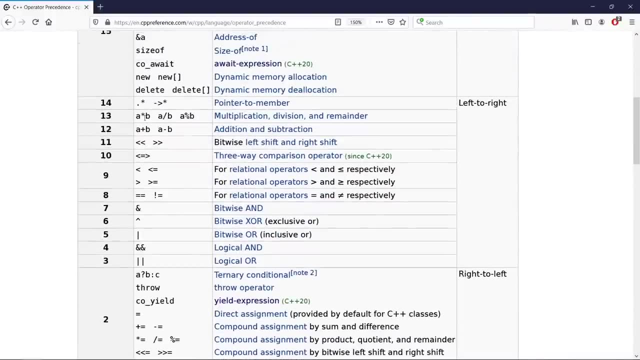 evaluated by our compiler first. another thing i want you to notice in this table is this column here on associativity. if you go back to our familiar operators here, you're going to see that these operators are left to right, so you should start evaluating things from left to right. but 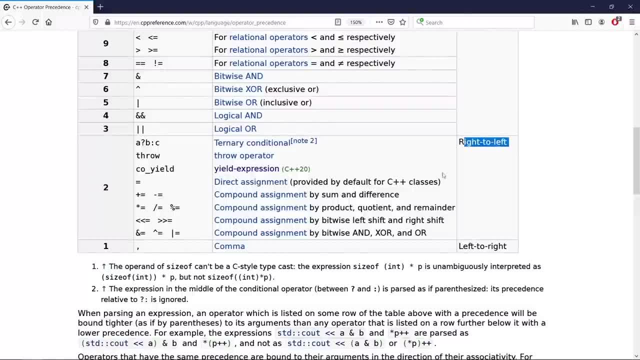 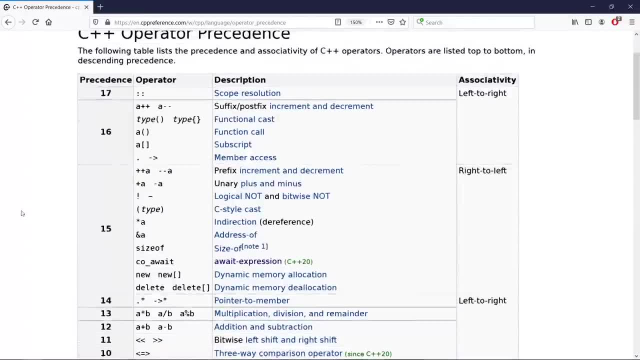 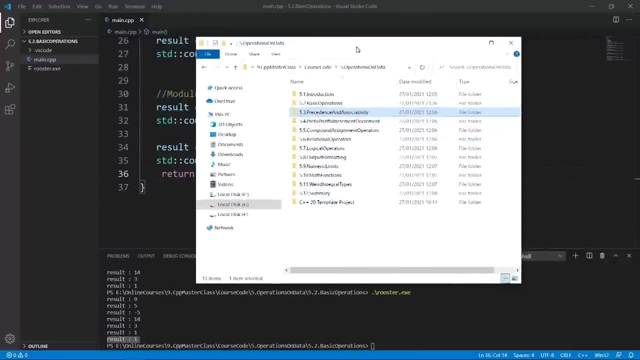 some operators have right to left associativity- and when we get to these operators, you will start doing things from right to the left. okay, i think it is time we went to visual studio code and actually played with these things. here we are in visual studio code. we are. 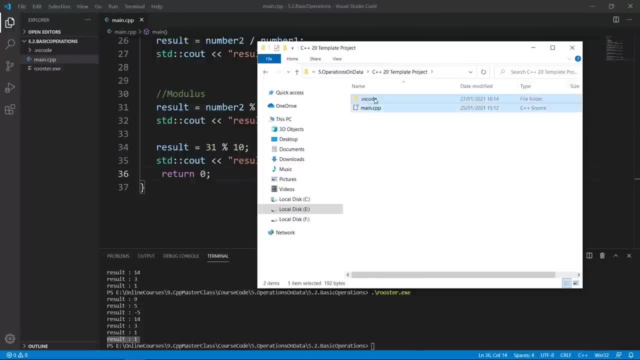 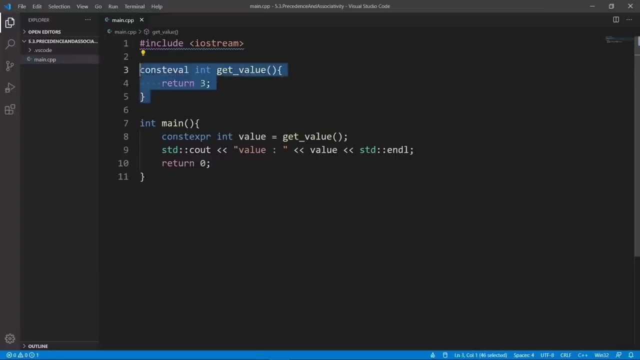 in our working folder. we are going to grab our template projects. we're going to copy this and put that in our lecture on precedence and associativity. we're going to put that in here. we are going to open this project in visual studio code. we are going to get rid of things. 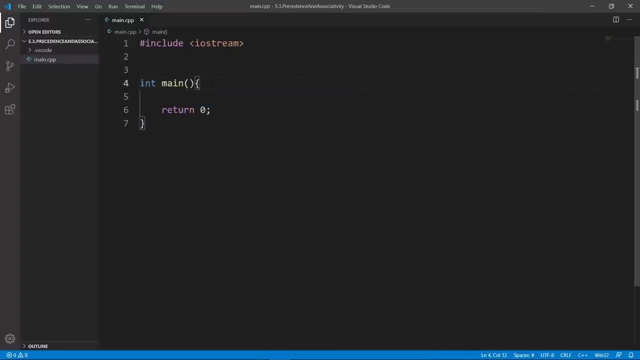 we don't need and remove this here in the body and we are going to put in our test code so that we don't have to type this and save on time. we have a few variables here- a, three through g, and we have an expression here or a statement that is combining multiplication. 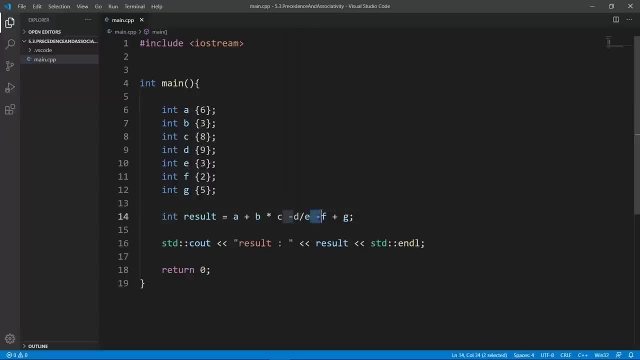 division, addition and subtraction, and we have to figure out which operation we're going to do first. i would challenge you to do this in your mind and try to guess what the result is going to be before we run this in our compiler. we're going to compile this with gcc and we are going to open. 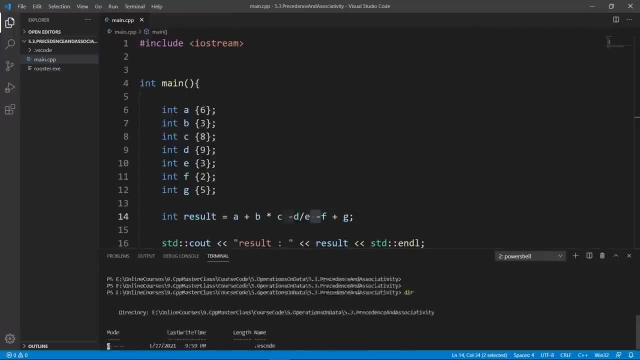 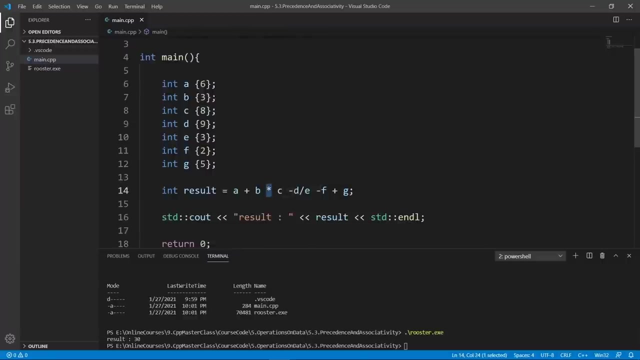 our terminal here, and if we do there, we're going to see that we have roosterexe. if we run it, we're going to see that the result is 30. how did we come up with that? well, the precedence and associativity table says that multiplication and division have to be done first, before addition and subtraction. 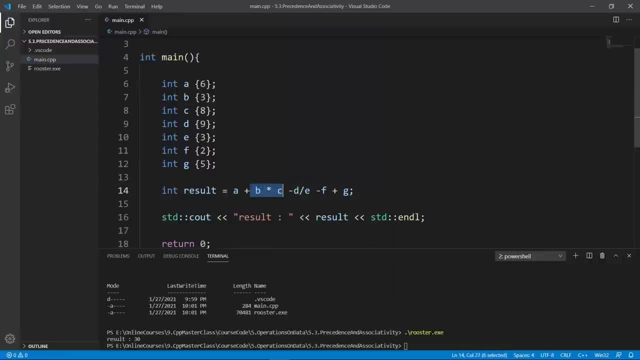 we are going to take b and c and multiply those. so, b and c multiplied, we're going to get a 24. we're going to try and do this in our brain. d divided by e- we're going to do that. so d divided by e, we're going to get a 3. so we're going to have a 3 here and after we have this, we're going to do: 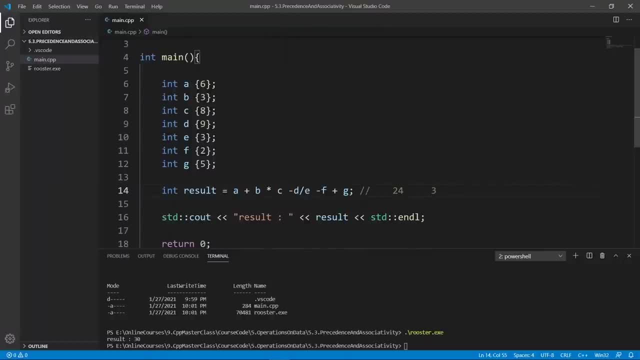 addition and subtraction. so we're going to take a and add that to the result of b and c. so we're going to say 6 plus 24, which is the result of b and c. we're going to minus the result of d and we're going to do minus here. i hope you are following. and then we're going to minus f and 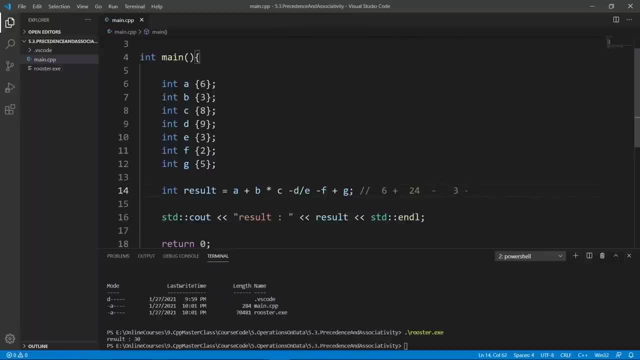 plus g, we're going to minus f, which is 2, and do a plus g, which is 5. okay, so this is our expression here and now that we have this, we have to think about how we're going to do this. we can try to do. 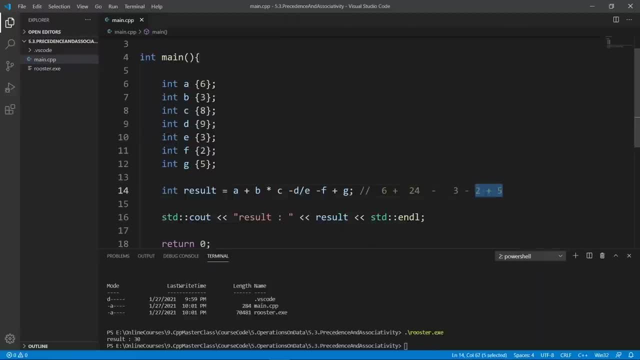 this from the right, do 2 plus 5, and then do 3 minus 2 plus 5 and go from right to left. so we're going to start from the left. but our associativity table says that addition and subtraction have left to right associativity, so we will start from the left. so we're going to do 6 plus 24, we're going. 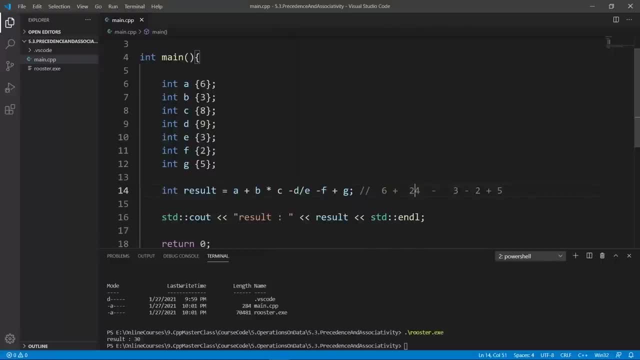 to get 30, we're going to minus 3 and we're going to get 27, we're going to minus 2, we're going to get 25, we're going to add 5, we're going to get 30. i hope you are following and we are really. 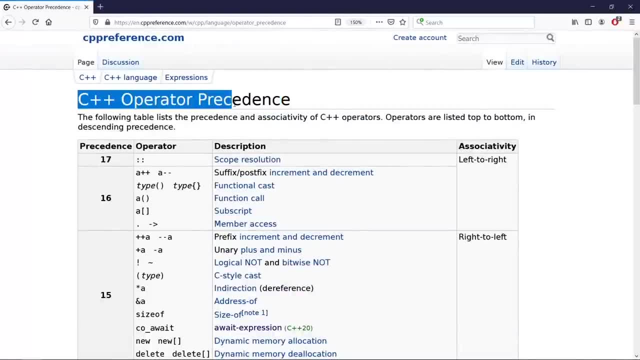 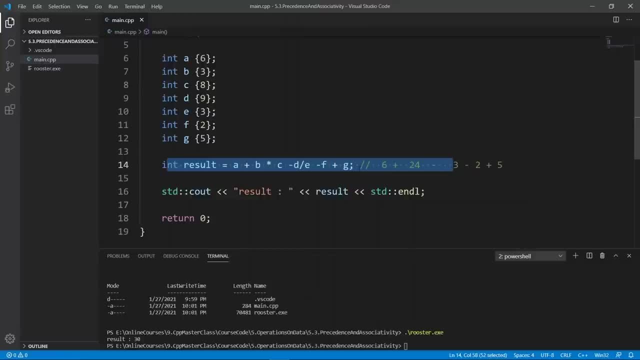 following the rules from our c plus plus operator precedence table here. okay, so this is really how you would use this precedence and associativity rules to evaluate your expressions. okay, here i have another example for you. so try to evaluate what we're going to get from this expression. here we have a divided by b divided. 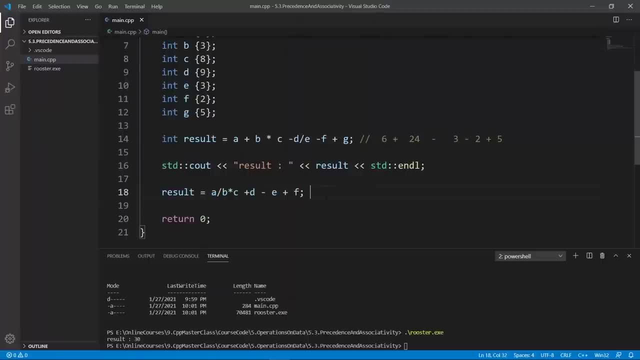 by c plus d, minus e plus f. try to do this in your brain and try to guess what we're going to get from the compiler if we print this out. we're going to put in our sddc out statement here and we're going to try and weld this with gcc. 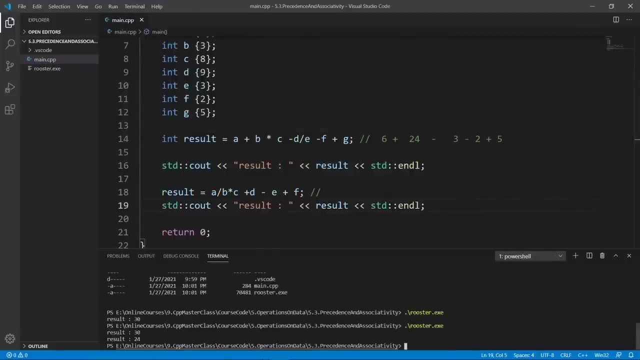 of course we're going to run rooster and you're going to get a 24, so how did we come up with that? we're going to start by division and multiplication. and again, where do we start? do we do b and c first, or do we do a and b first? well, we can check our precedence table here. 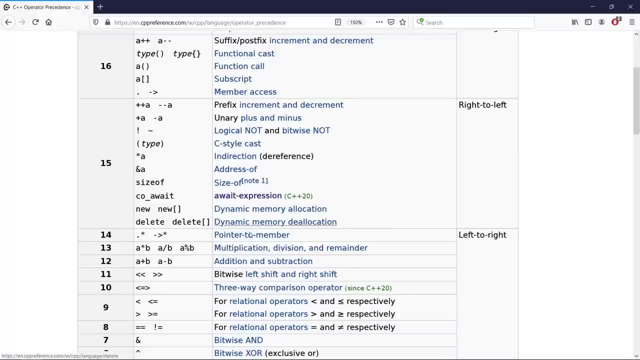 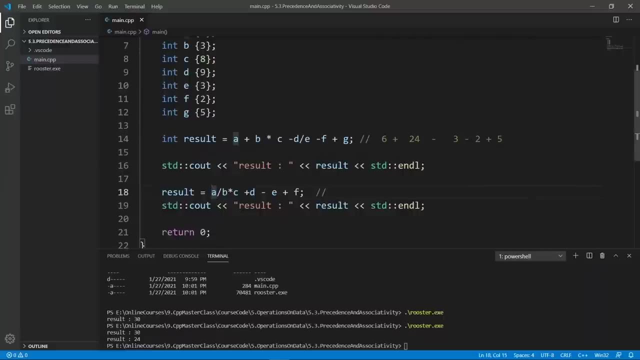 and we're going to check the associativity of multiplication and division. we're going to go to this entry here, 13, and we see that it is left to right associative. these operations here are left to right associative. so what we're going to do, we're going to start from left and go to right. so 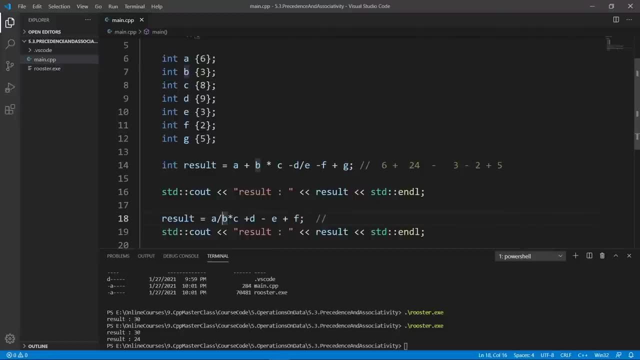 we are going to take a and divide by b. if we take a divided by b, we're going to get it too. so let's type that here. then the result of that is going to be multiplied by c, and if we go up we're going to see that c is 8. so we're going to multiply by 8. 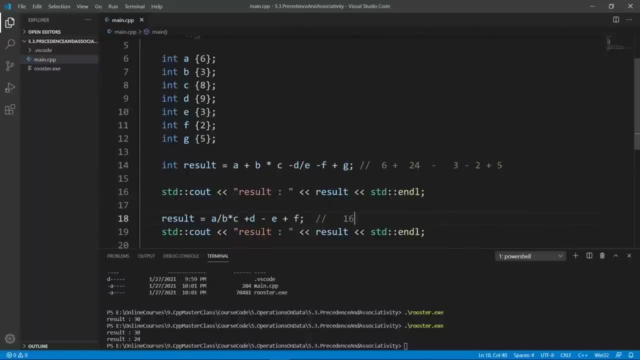 and get 6, so we can replace this with a 16, and we should be here- then we're going to add d- d is 9, then we're going to subtract e, which is 3, then we're going to add f, which is a 5.. so we have 16. 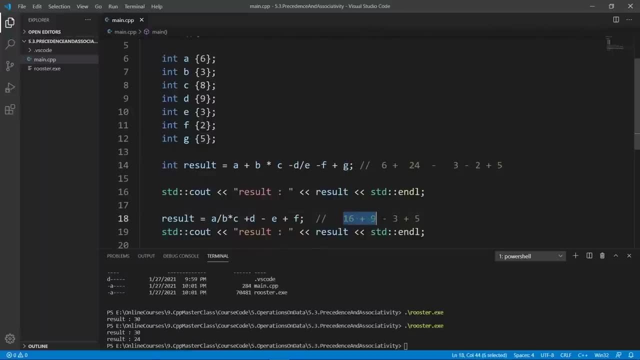 plus 9.. this is going to give us 25.. minus 3.. okay, by checking this out, i see that i made a mistake. f is not five, it is a two we have here, and if we do this from left to right because addition. 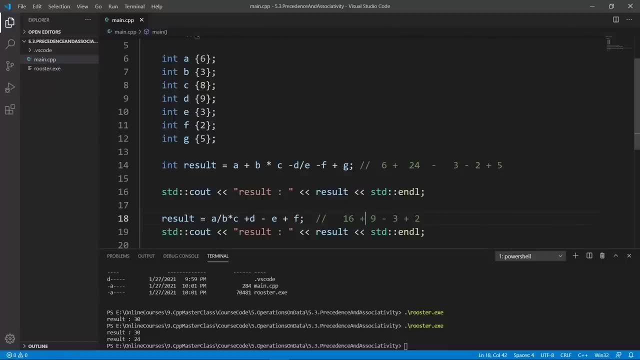 and subtraction are left associative. we have to do them from left to the right. we're going to take 16 and add a nine. we're going to get a 25 minus three. we're going to get 22 plus two, we are going to get 24 and that's what we have here. i really hope this makes sense. 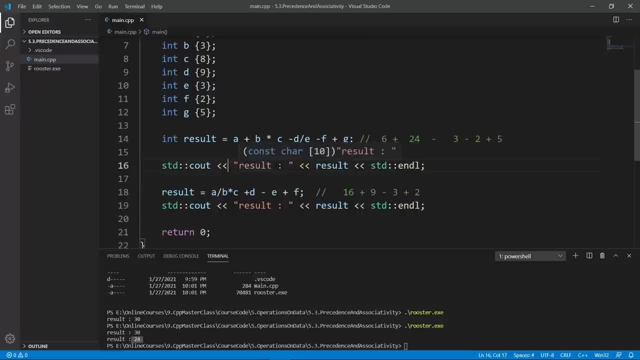 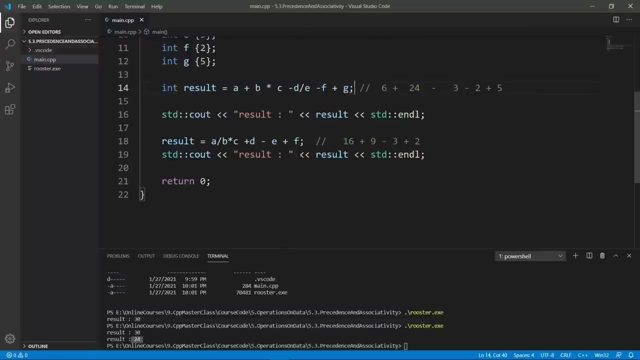 okay, so we have seen how we can use this precedence table, but sometimes you want to make it really clear which operations should be done first, and you can do that by using parentheses around your expressions. let's grab the first expression here and do it again. we're going to. 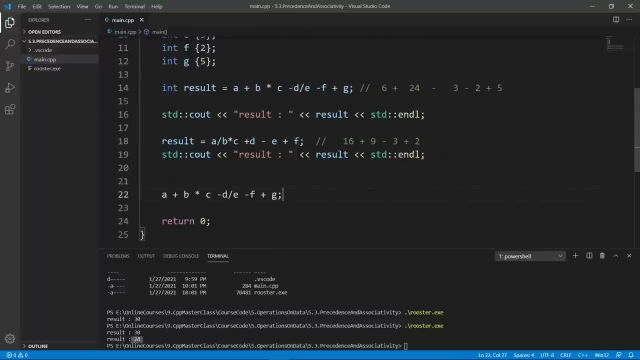 copy it and go down and put that in place and we're going to store the result in our result variable and notice that we are reassigning these things to the result variable so that we don't have to declare another variable. I think this is clean and that's what we're doing here. so what we 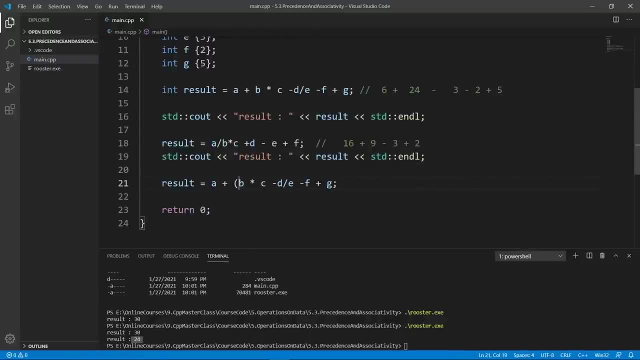 can do here is make it clear that we want multiplication done first by using parentheses, and make it clear that we want the division to be done first. and when you do this, the compiler is going to see that you want this application operation here done first and that's what it is going to do. and if we print reserved again, we're. 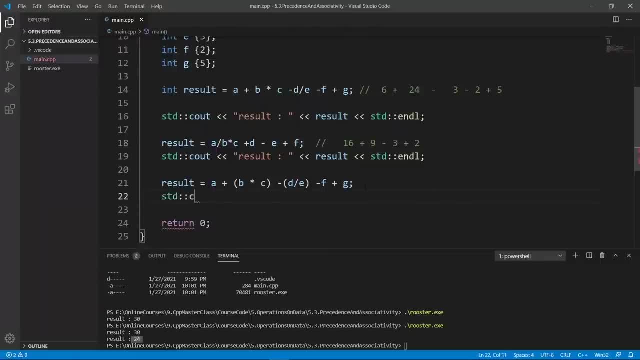 going to get exactly the same thing we had before: stdc out result- and we're going to put result out and let's make it clear that we are using parents here to signal which operation we want to be done. first. we can compile this with gcc. we're going to run the task to build with gcc and if we run 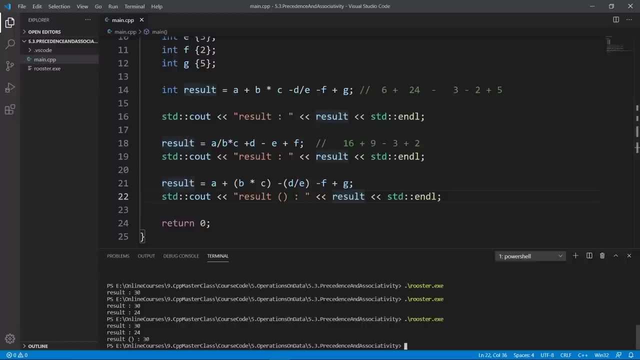 the program. we're going to see that the result is 30, exactly what we had before. but now it is very clear to the reader of this piece of code that we want b and c done first. they don't have to go through the precedence table to really try and figure this out, potentially wasting precious 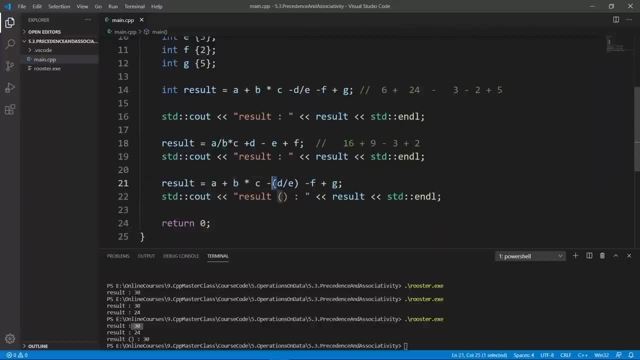 time. another thing you can do with this is, for example, what if the precedence table is not working according to your needs? for example, you really want a and b done first. you can specify this with parents here, and what this is basically going to do is going to force the compiler to do this first. 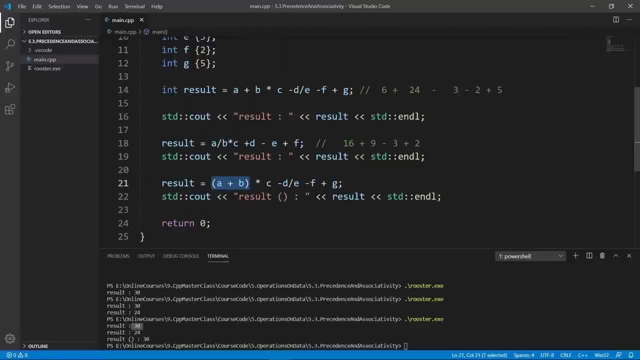 it's no longer going to do b multiplied by c and d divided by a. it's going to evaluate this first, then it's going to follow the order order in the precedence table that we have seen before, so try to guess what we're going to get now, and 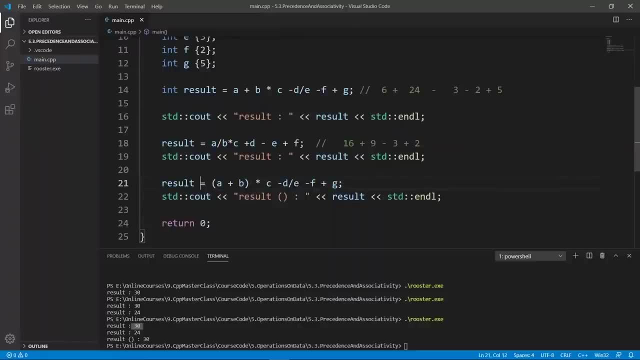 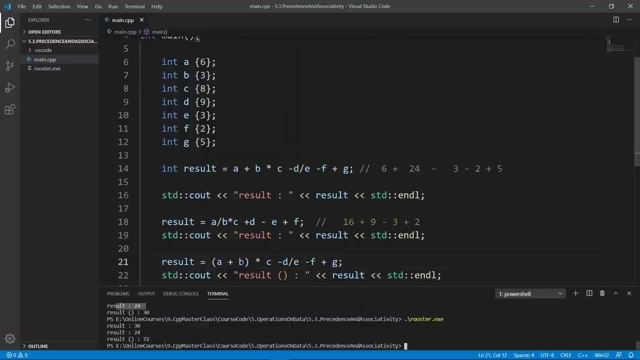 i am going to run the code and we're going to go through this together. so let's run task and we're going to run rooster. now you see that the result is 72. what is happening here? well, let's go through this line by line. we are doing a plus b, which is a nine, so we're going to get a nine. here we're. 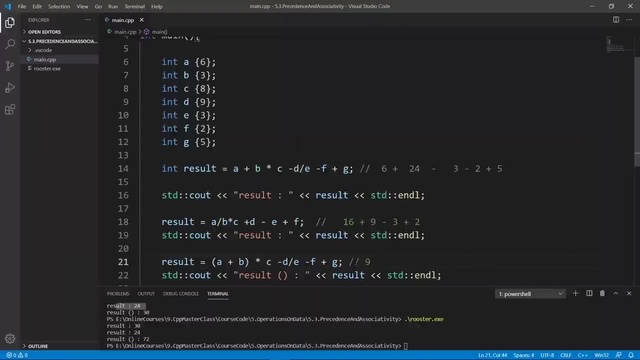 going to put that here. as a result of this, we're going to run the task and we're going to run the a comment. then we're going to multiply that by c, so we're going to do 9 multiply by 8 and that's going to yield a 72 and by that time we're going to be here and we're going to do the division first. 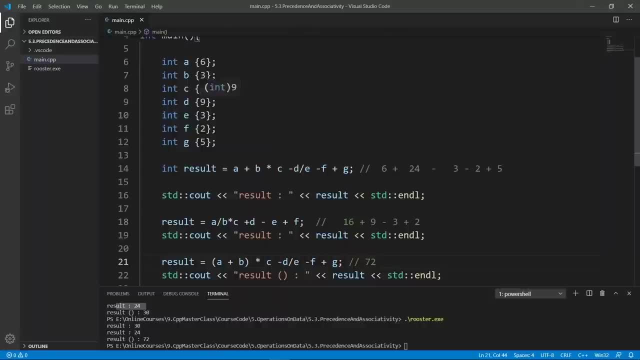 d by e. then we're going to take 9 and divide by 3. that's going to yield the 3. so we're going to have a 3 here minus 3. we're going to minus f, which is a 2, and we're going to do plus g, which 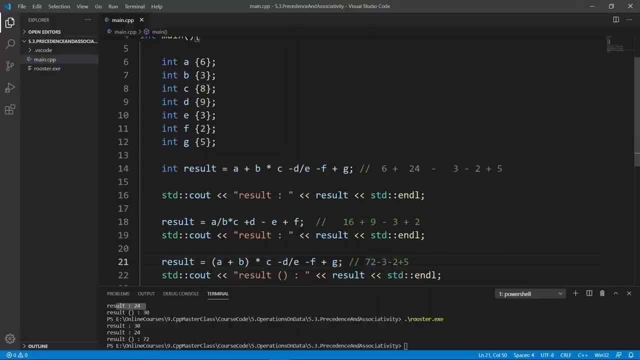 is a 5. if we evaluate this, we're going to get 72 minus 3, which is going to be 69 minus 2, it's going to be 67 plus 2, it's going to be 72, and that's what we have here. hopefully you can see that. 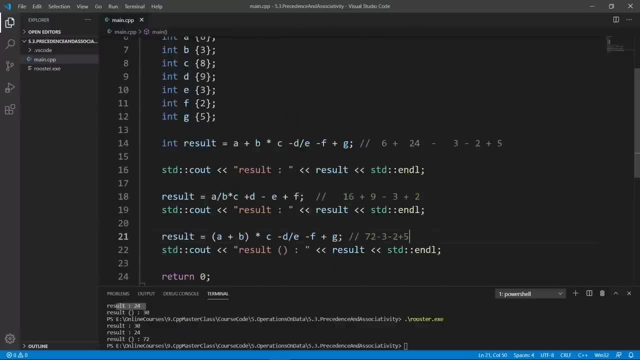 using the parents. not only can you make it very clear which operation you want to be done first, you can also define the rules that are prescribed by the precedence tables that are defined in c plus plus. i hope this makes sense, and this is really all we set out to do in this lecture: to learn a. 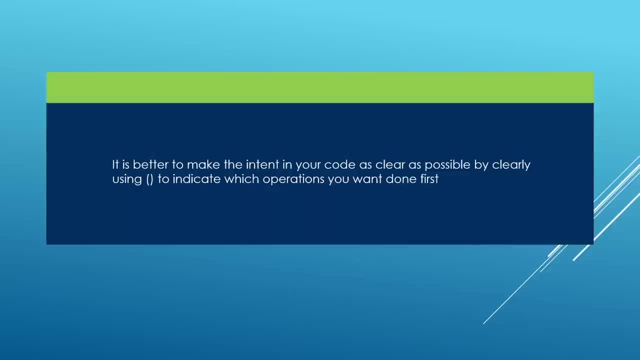 little more about precedence and associativity, and my advice to beginning programmers is not to rely on the precedence table too much. it is to try and make your intent very clear using parentheses, and anyone reading your code won't have to go check these rules in the reference C++ documentation. they are going to directly understand what your expression. 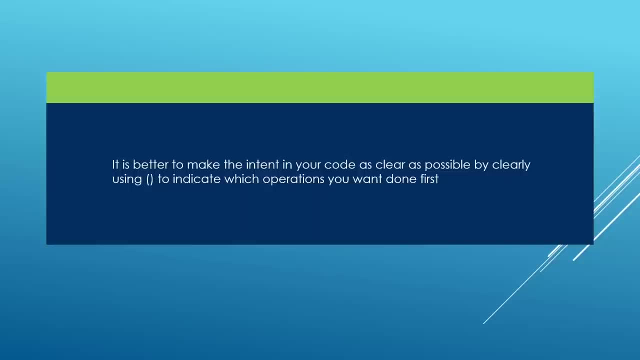 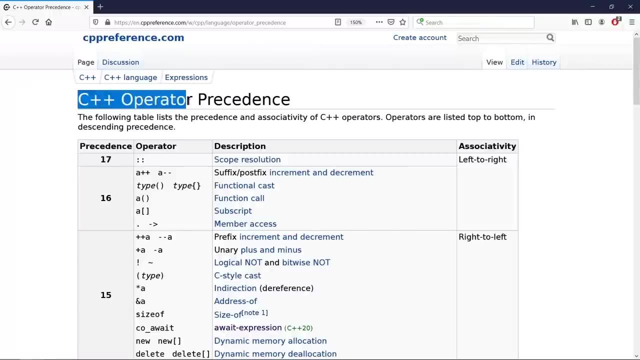 is going to do, and that's a good thing. readability of your code is really something you should strive for. this is really all we set out to do in this lecture. I hope you have a better idea about precedence and associativity. we are going to stop here in this lecture. in the next one we're going 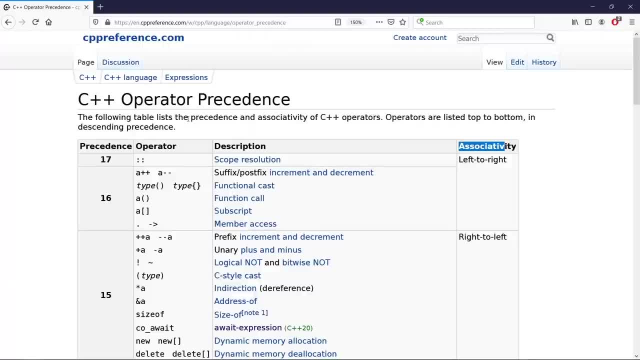 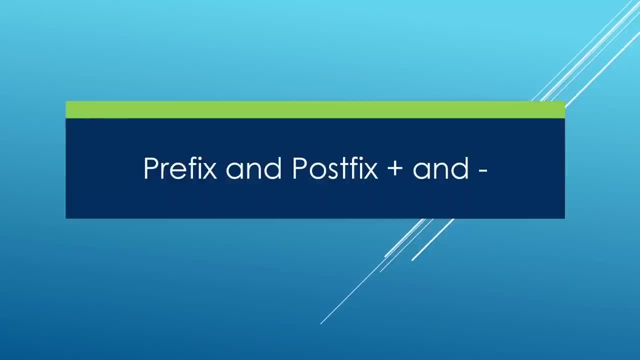 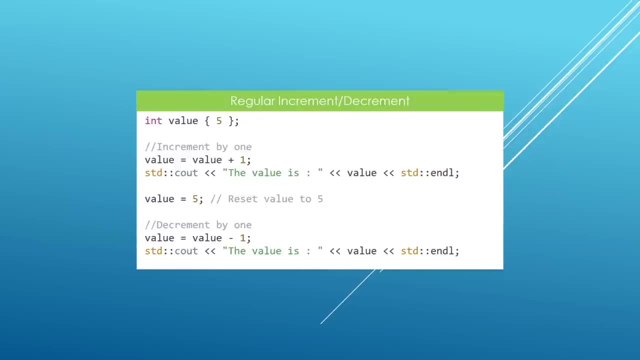 to learn about some cool things we can do with addition and subtraction. go ahead and finish up here and meet me there. in this lecture, we're going to be learning about prefix and postfix, addition and subtraction. we have an example here, and it is a simple example. we have seen a lot of times by now. 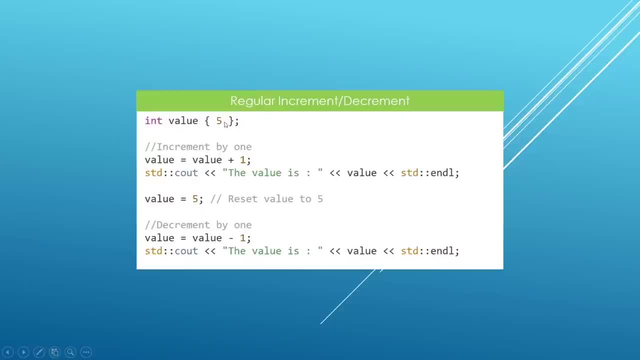 we have a variable value- it is an integer- and we have a five inside. we can add a one to it or we increment it by one. this is another term we use in programming languages. when we say we are incrementing the value, we are adding something to. 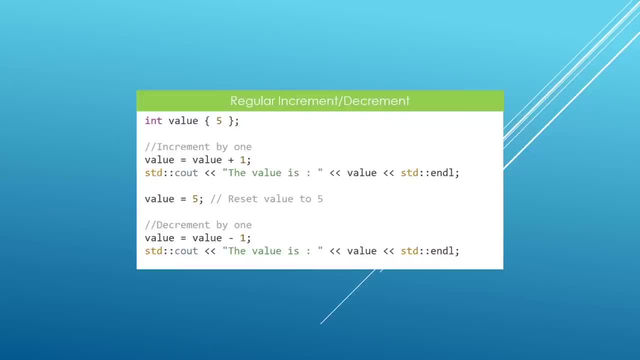 it. in this case we are incrementing it by one and we are basically going to store a six in this value here. so if we print this out, we're going to get a six here. this is what we would expect. we are resetting the value to five and we are going to minus one or decrement by one, and the result is: 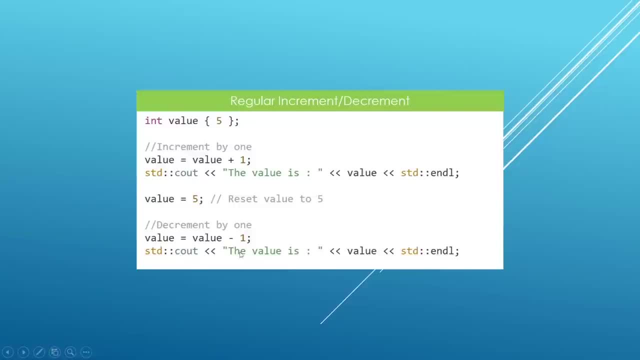 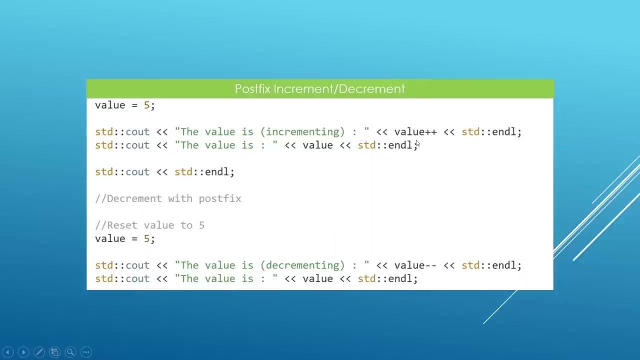 going to be saved in value again. so the second stdc out statement here is going to print a four. this is something you should expect. now, another thing we can do in c++ is do something like value plus plus here. and what do we mean by that? when you use a postfix increment operator like this? 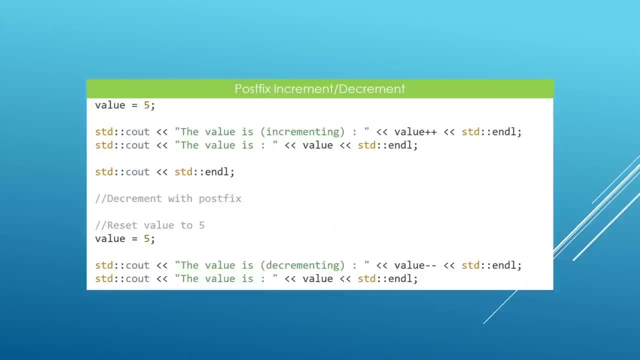 the first thing you should know is that this is going to increment by one. it's not going to increment by any other value. c++ doesn't provide a way for you to specify another number to increment by. so value plus plus here is going to increment by one. but another thing you should know is that it's not going to increment. 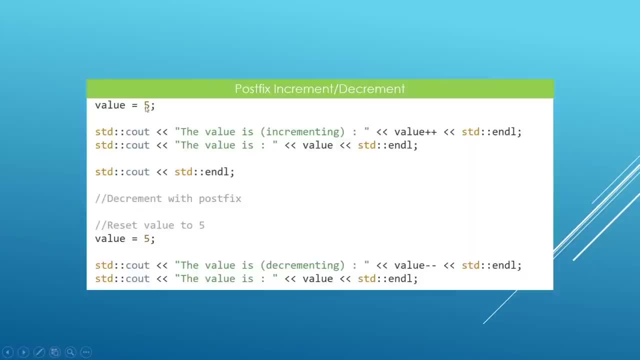 directly what's going to happen here. if you look to the top here we have a value five. when execution hits this stdc out statement, we are going to grab the value here. so here we're going to really print a five, but as soon as this statement. 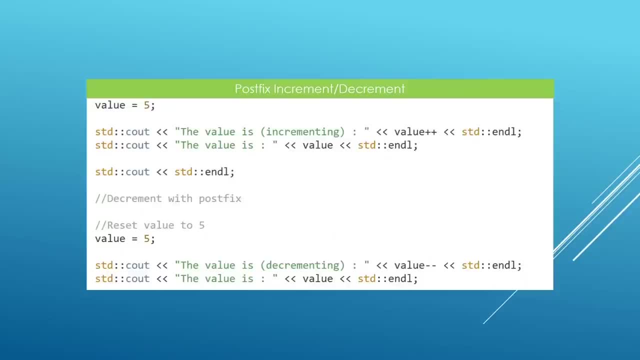 is done, the value is going to increment by one. so the next time somebody is going to use this value here is he's going to find in a six and that's what we have here. so the first one is going to print a five because we're going to grab the value in here as is. but as soon as we have our value, 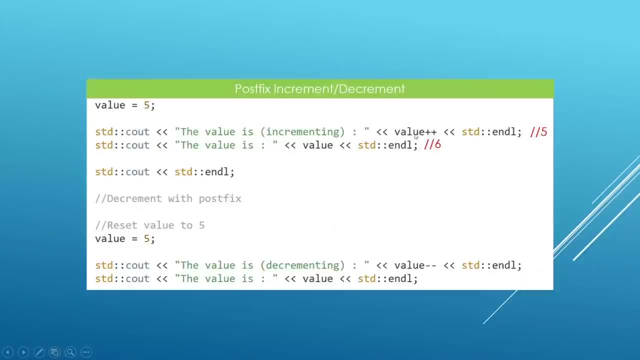 this is going to increment by one. this is what we mean by this value plus, plus here. and uh, the second statement is going to print a six because it is already incremented. and we call this post fix increment because plus, plus is after the value here. and this is really what. 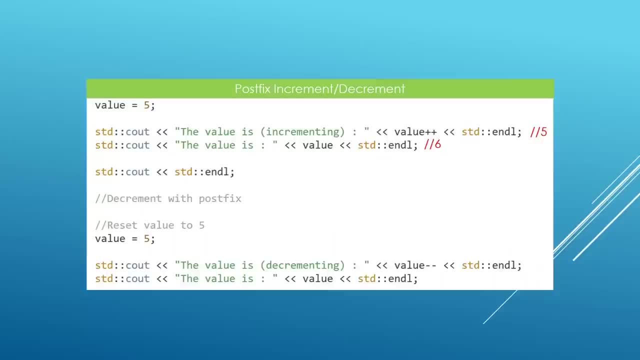 this operator does, and sometimes it is going to come in handy in your c plus plus applications. we can also do the same thing with minus minus. it is going to grab whatever value we have in this variable. so we have in a five. so that's what we're going to print here. and the next statement: 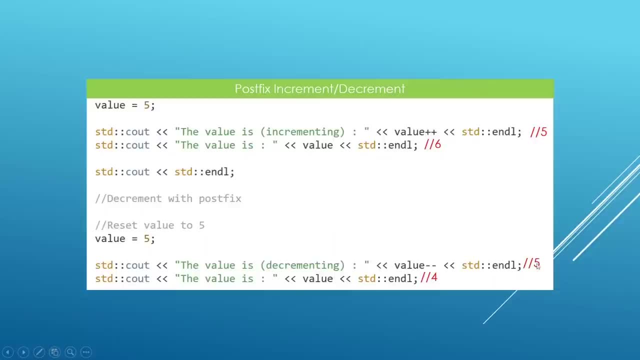 is going to find it already decremented by one, because after we have our five, we're going to decrement by one- that's what we are saying here- and we're going to find in a four, because five decremented by one becomes a four. i really hope this makes sense. okay, so what? 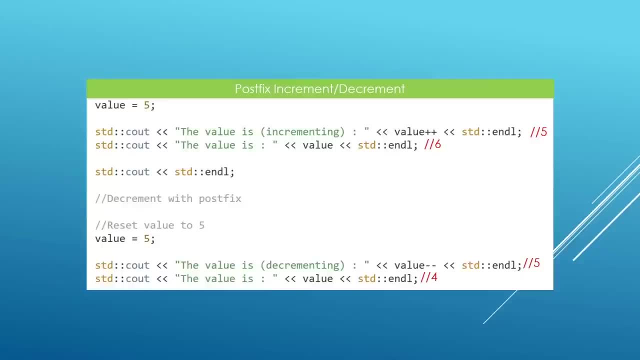 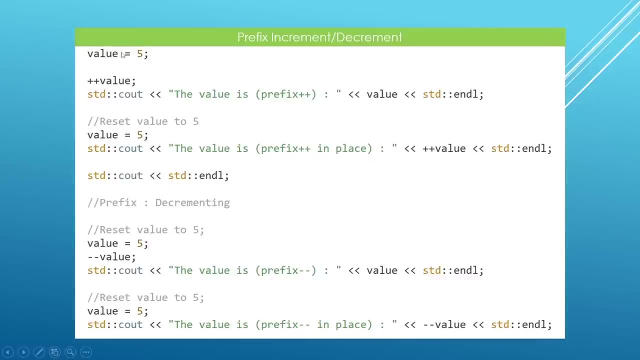 we have seen here is post fix, increment and decrement. but we can also do a prefix version of this thing. if you look at the example we have here, we have a five and we are saying plus plus value. so this is going to increment the value directly into the state invested as one. so as soon as this statement is executed, the plus plus value statement. 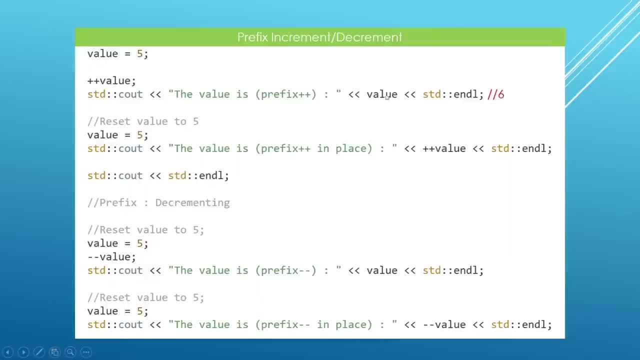 here we're going to have a six inside and if we print it we're going to get a six. and this is what you see here. if we go down, we are resetting our value and we are going to prefix increment in place. so in here we are going to increment the value before we actually print it here. 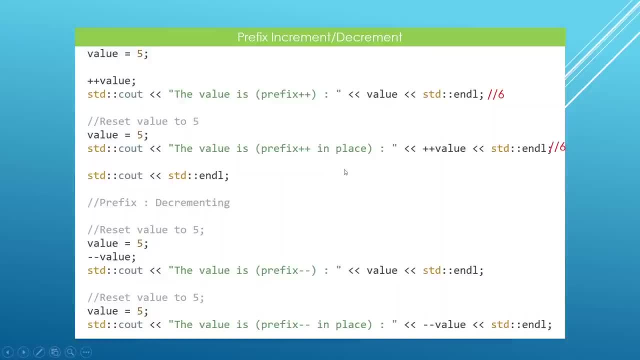 and we are also going to get a sixth year. i hope this makes sense. you have any problem with this. i think if we go in visual studio code, you're going to have a better way to say this. you're going to see the code running and make sense of it. 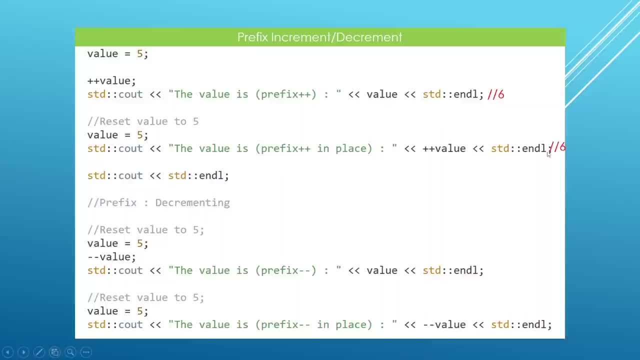 okay. so i think that now you understand why we're going to have these numbers printed if we go down. we can do the same thing with decrementing. we have a value here, it's five. if we prefix decremented, it's going to be a four here, and if we print it we're going to get a four if we go down. here we 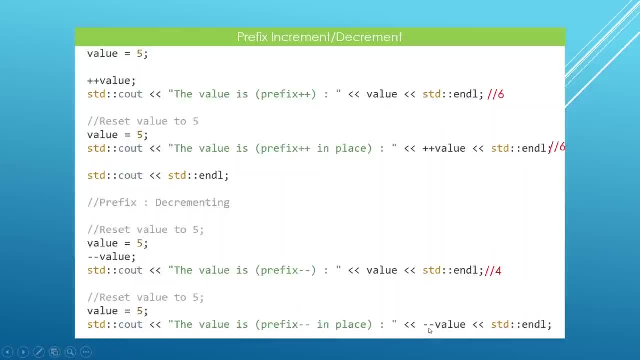 are resetting that to five and we are going to prefix decrement in place and, uh, this is also going to print a four, because we have a five here and if we decrement it by one, we're going to get a four, and that's what we're going to get here. okay, this is really all these prefix and post. 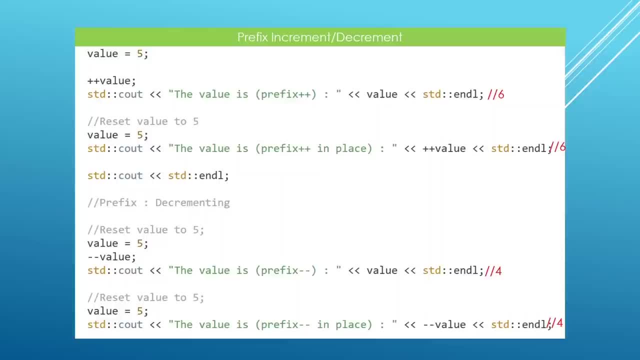 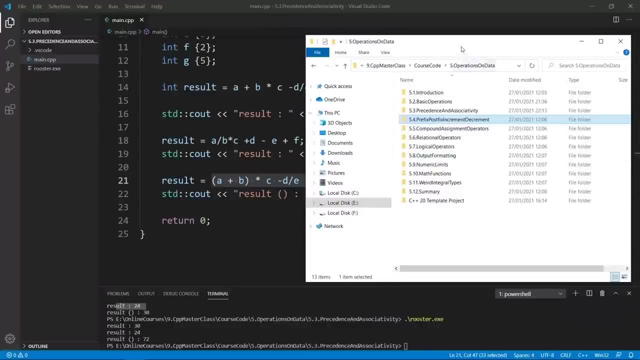 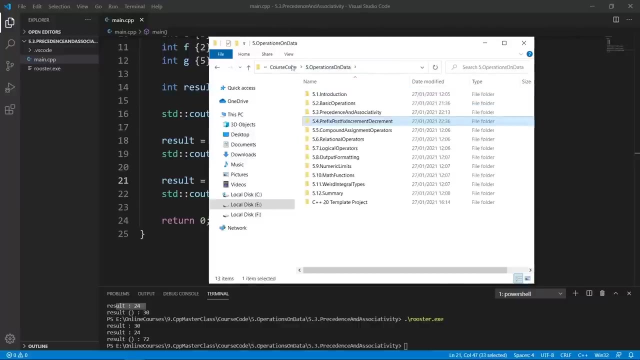 fix, increment and decrement operators are about. we are going to go in visual studio code and actually see this running. okay, here we are in our working directory, going to do the usual. we're going to copy code from our template project. we're going to put that in here. we're going to go up and open this up in visual studio code. so we're going to remove. 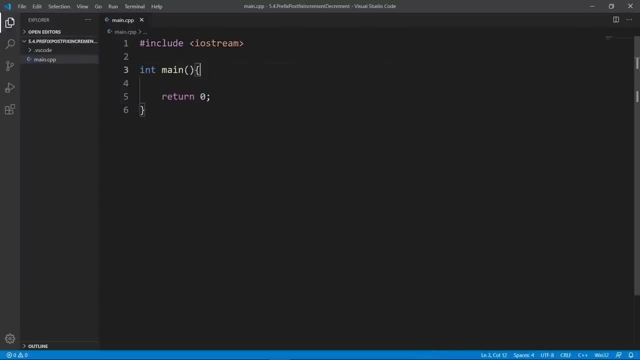 things we don't need and we're going to remove this and we are going to put in the code we exactly so in the slides here we have a value. it is an integer and it is five. if we increment it by one, we're going to get a six here. okay, and if we print it, that's what we're. 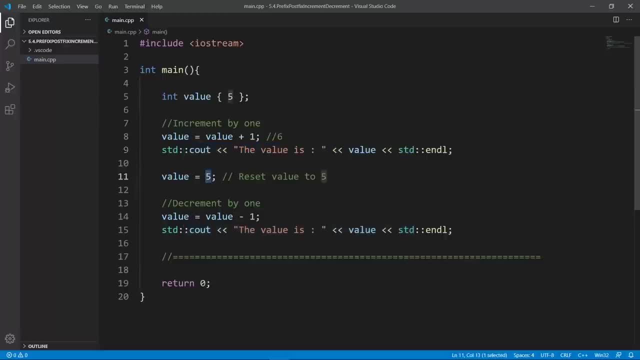 going to get. we are resetting this to five and if we decrement it by one, we're going to get a four here. so if we run this piece of code, we should have a six here printed out and a four down here. we're going to bring up our terminal and build this with gcc. the build is going to go through. 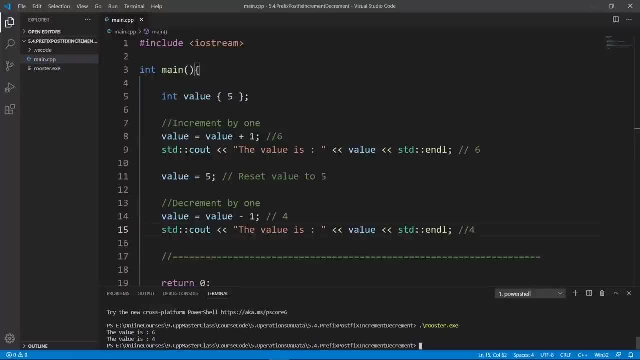 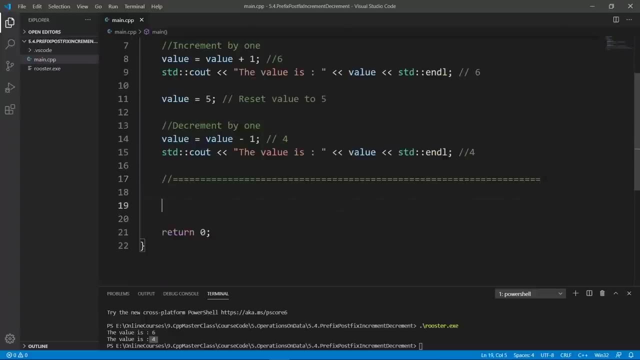 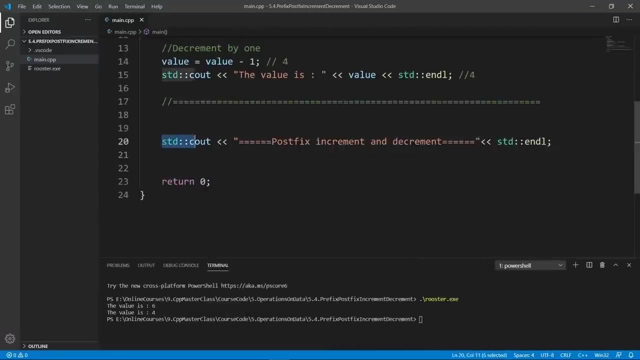 and if we run the program we're going to get the value is six and it is four, and this is what we expect here. okay, now that this is really clear, we're going to go down and play with post fix, increment and decrement. i am going to put in a separator here so that we can clearly see in our 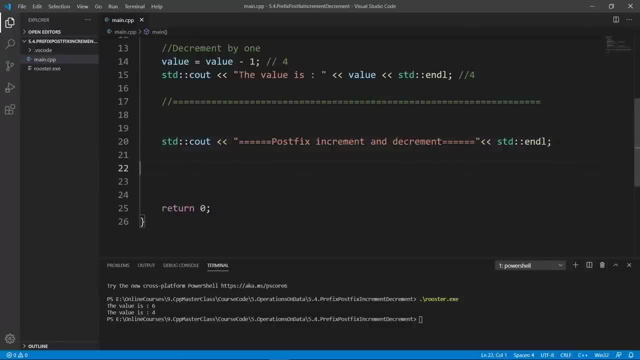 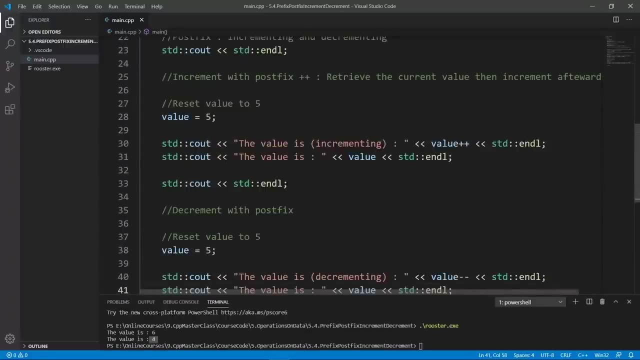 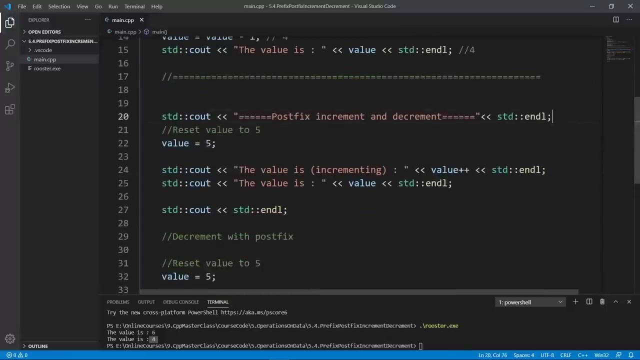 terminal here and we are going to put in our test code that we are going to use to play with this. let's bring this down a little bit so that you can see everything. we can remove these things. we don't need them anymore. okay, we are going to take the value we had, we're going to reset that to a 5 and if we value the 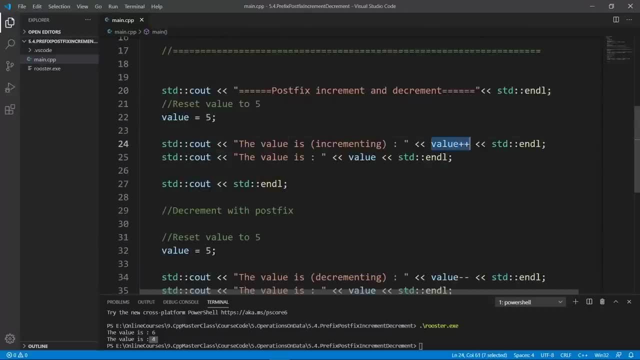 plus, plus. here this is going to be a 5 because we're going to capture the value as is. so here we're going to get a 5, but next time we get this value it's going to already be a 6, because we increment immediately after capturing the value here. so here we're going to get a 5 and here we're. 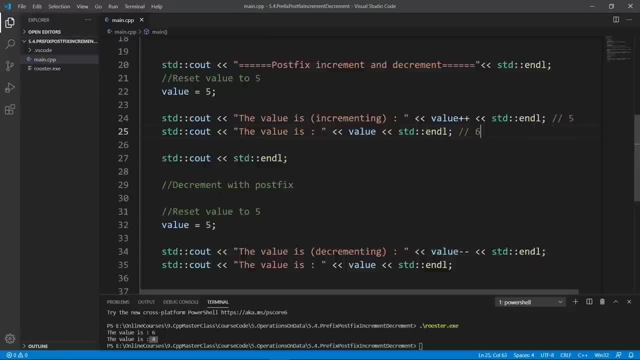 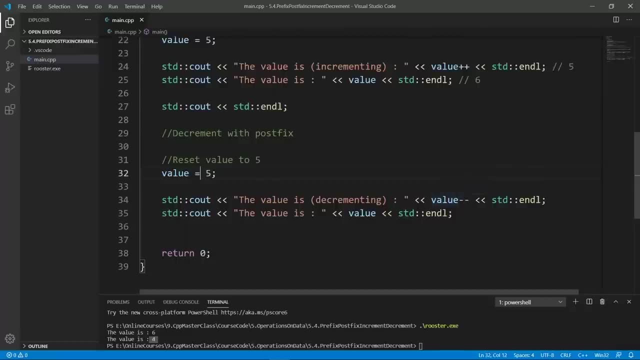 going to get a 6- i hope this makes sense- and if we go down here, we are resetting our value to 5 before we do any decrementation. we are going to capture the value as is because we are doing post fix decrement. and here we're going to get a 5 because we are capturing the value as s but as. 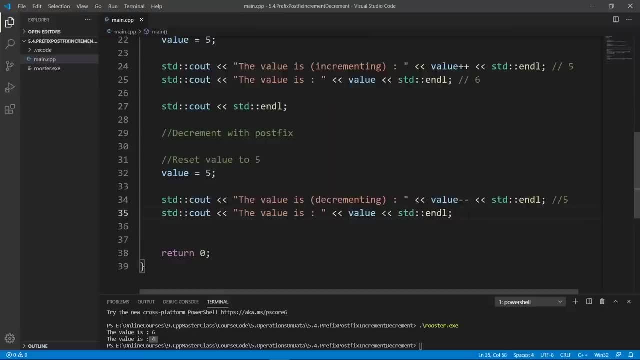 soon as we capture our value, we're going to decrement it, and the other statement here is going to get a decremented value and that's why we're going to get a 5, because we're going to get a 5 value and that's going to be a 4.. so here we're going to print 5, 6, 5, 4.. let's try and build this. 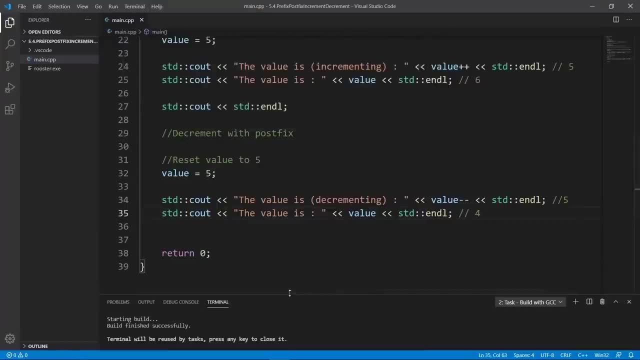 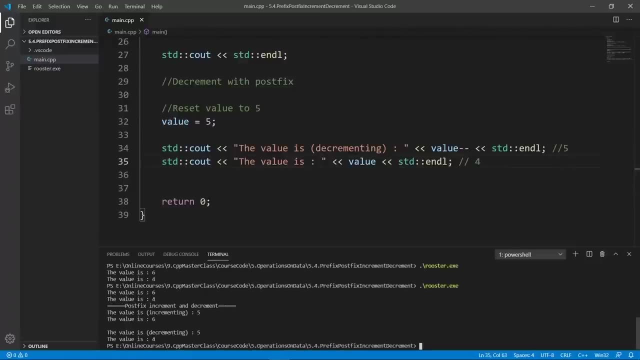 with gcc to see that we have no problems. we have no problems. the world is good. if we try to run rooster now, we are going to get the results we had before. but for this code we just put in here, the value is going to be a 5 and that's what we. 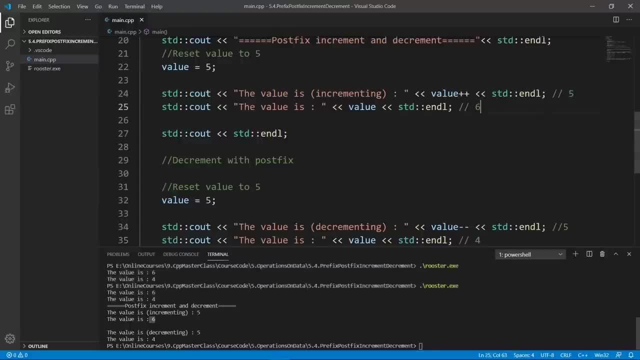 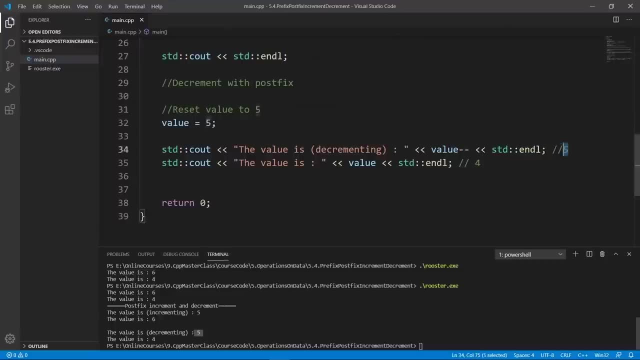 have here and we're going to get a 6, which is coming from here, after we are going to decrement and we are going to capture the value as is. we're going to get this 5 here and for the last statement, we're going to get a 4 because the value is already decremented and that's the 4 we 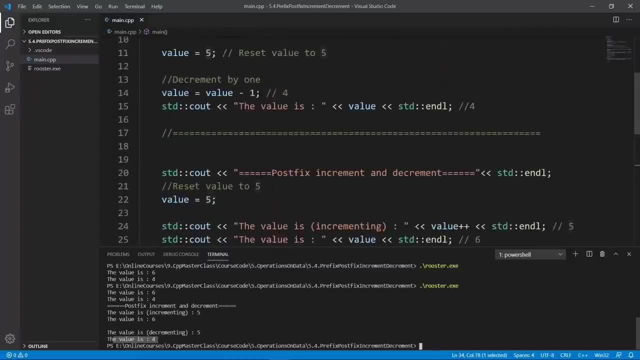 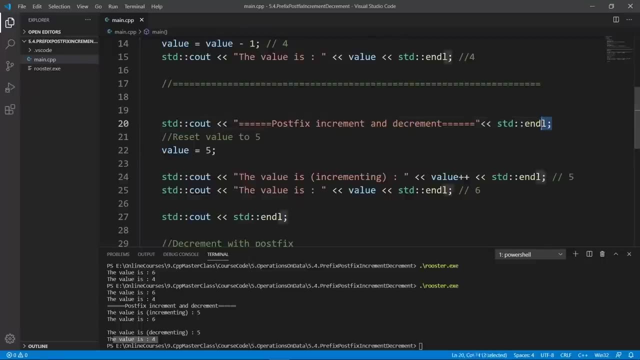 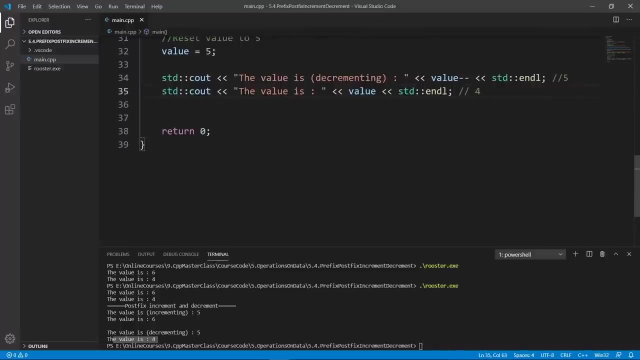 are seeing here. i really hope this makes sense and this really covers the post fix, increment and decrement operators. we want to see in this lecture is that we can also do prefix increment and decrementation. we're going to go down here and set up a place where we're going to be playing with this. 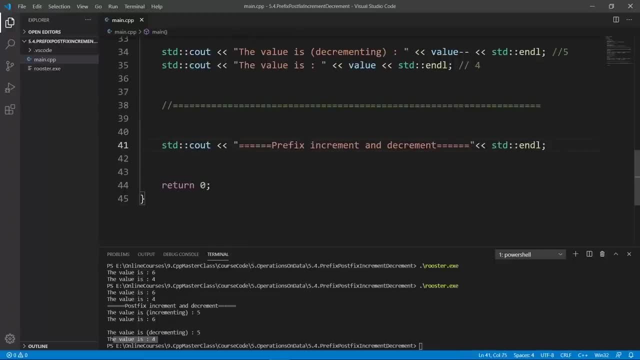 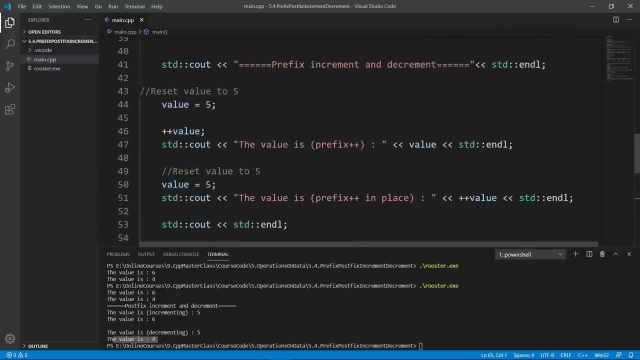 so we're going to say prefix and we are going to put in our code- because i don't want to type all this, that would waste your valuable time- but i do encourage you to type these things out and really drill them in your brain, because that's how you're going to learn. 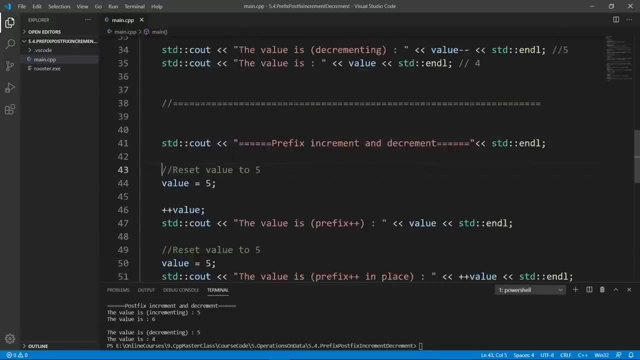 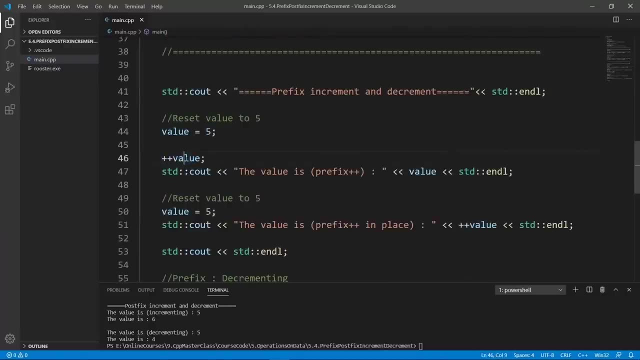 okay, let's bring this down so that we can understand this piece of code. so we are starting by resetting our value to five and uh, notice here that we do plus, plus value. this is going to increment value right away. by this time the value is going to be six and if we print it out here, we're going 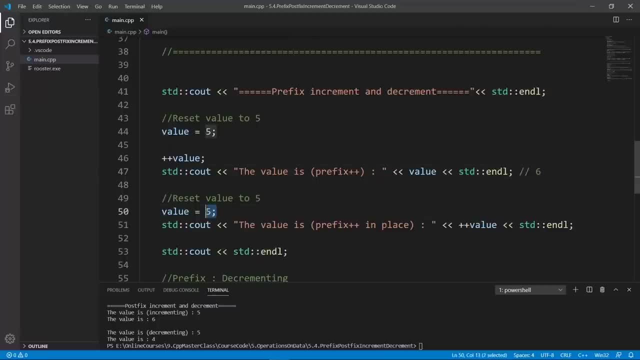 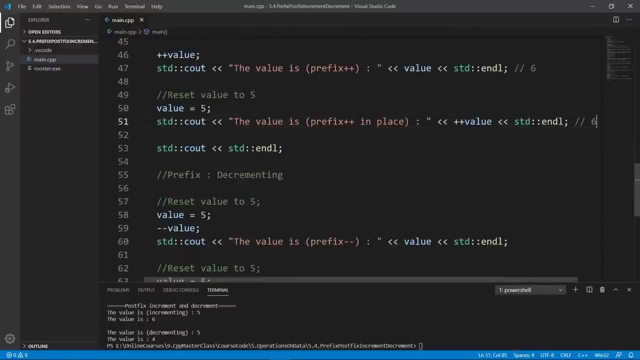 to have a six printed down, we're going to reset it to five and then we're going to increment that in place. this is also going to be printing six and if we go down, we're going to do the same version of the same thing, but we are going to be decrementing, so we're going to decrement. 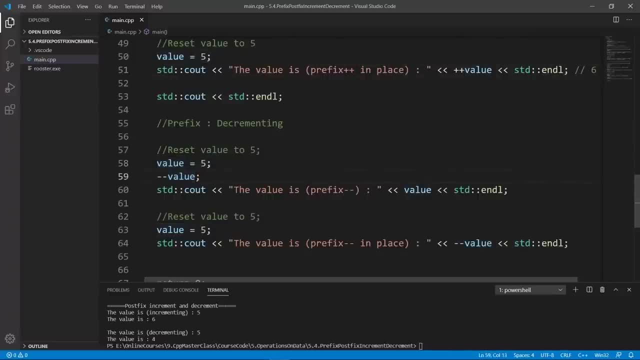 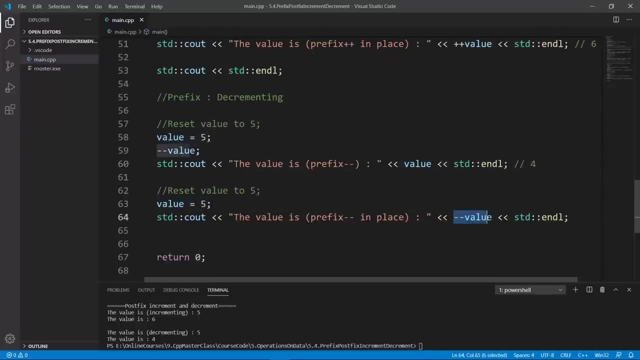 the value that we just reset here. here it's going to become a four, and that's what we're going to print. and if we go down here we reset it again to a five and we prefix decrement it in place. so the five here is going to become a four in here, and that's what we're going to print. 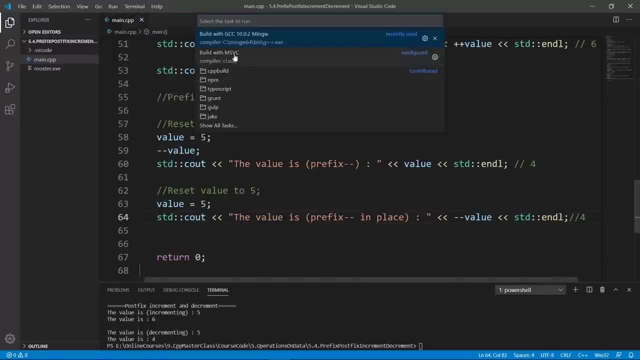 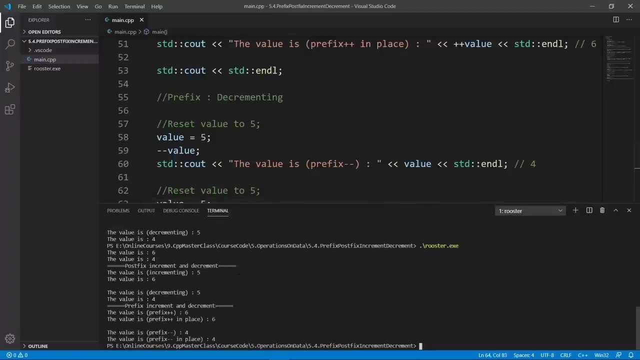 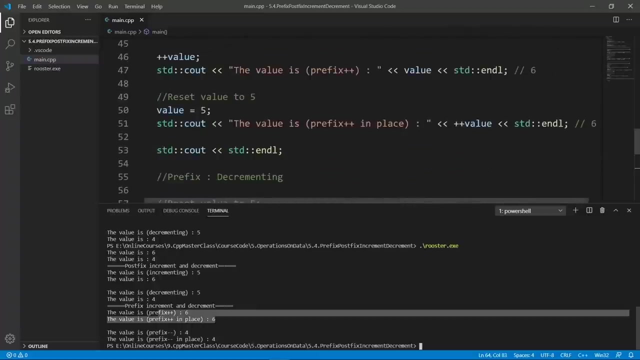 out. if we build and run, that's what we're going to get. we're going to run our task to build with gcc, this good- and if we run our rooster application, the research for the code we just put in here are just going to show up here and you see that we get a six, six. this is six, the other six and 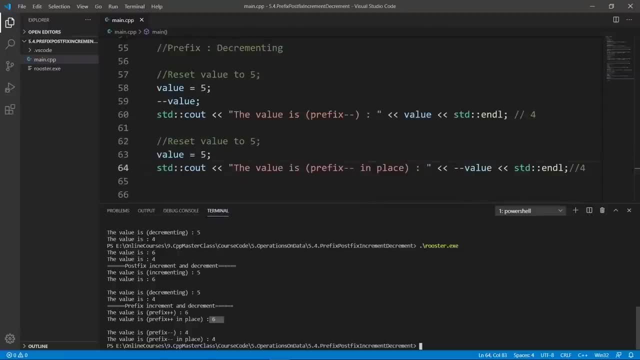 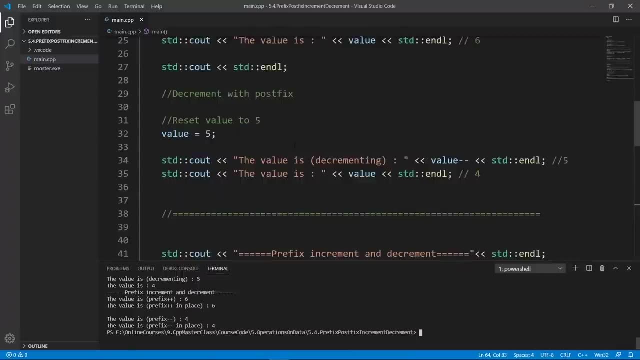 for the last two statements. we're going to be getting fours, and that's what we have here. i really hope that now you have a better idea of this prefix and post, fix, increment and decrement operators and you're going to make use of them when they really help you design your applications better. okay, so these are your tools. use them when. 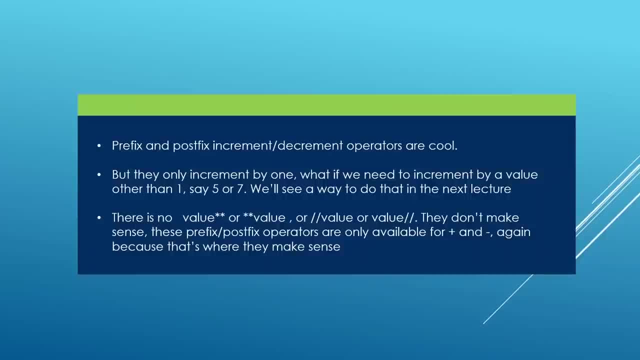 they make sense. another thing that i want to emphasize here is that these operators only increment or decrement by one. you can't make them do things in increments of five or seven or ten. they are going to work in increments or decrements of one. we are going to see a way we can do that. 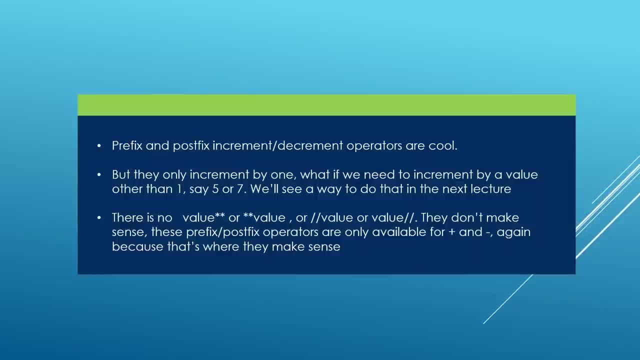 with other operators in the next lecture. but this prefix and post fix operators can't do that. and another thing that some of you might be wondering about is if we have the same kind of operators with multiplication or division and we don't have those operators in c plus plus. maybe you're going to have them in the future when they make sense. 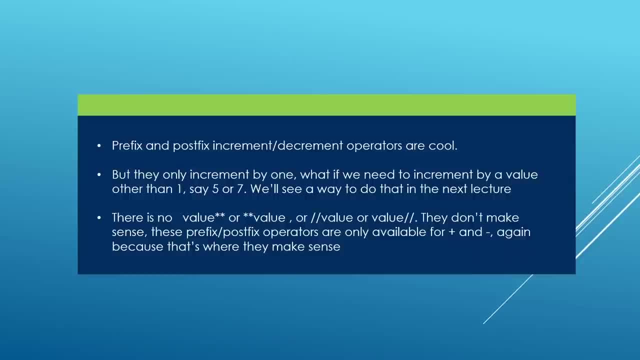 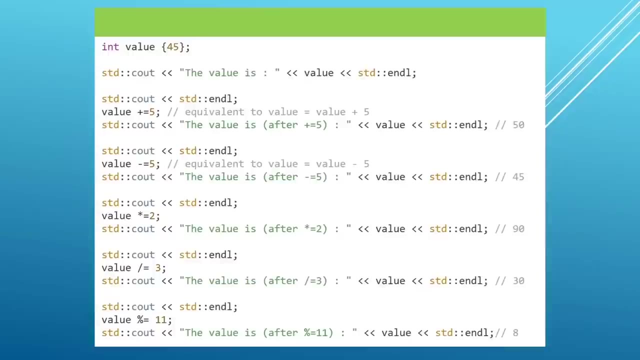 but in the current version of c plus plus we don't have them. we are going to stop here in this lecture. in the next one we're going to learn about compound assignment operators. in this lecture we're going to learn about compound assignment operators, and these are operators that allow you to do an 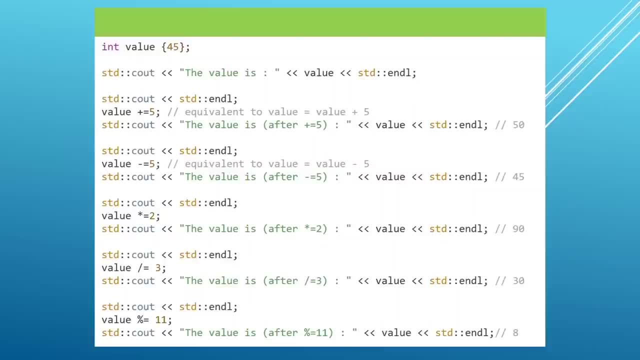 arithmetic operation like addition, subtraction, multiplication, division and modulus, and assign the result to a value in one go. let's look at an example here. we have value here which is 45. it is an integer and we're going to print that out. but if you go down here, we are doing value plus e. 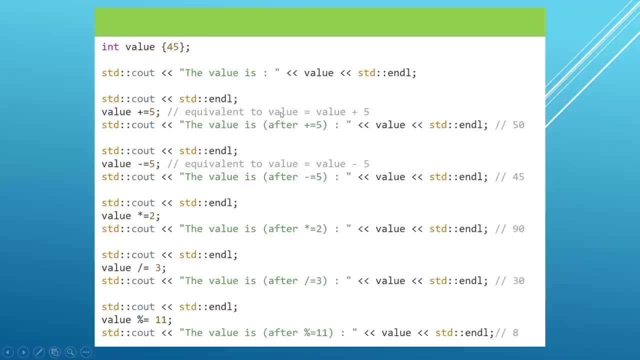 plus five and if you look at the comment here, this is equivalent to if you did: value equals value plus five. so what this is going to do, it's going to take whatever value is in this value here. it's going to increment that by five, so that's going to become a 50 and we're going to store. 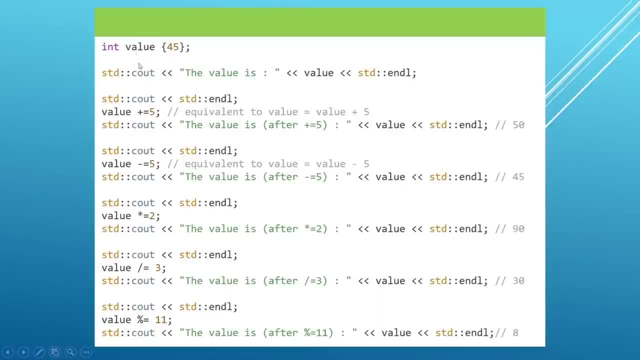 that 50 results back in this variable here. so by this time, if we print this out, we're going to get a 50.. again, we're going to take the value: it is a 45. we're going to add a 5. it's going to. 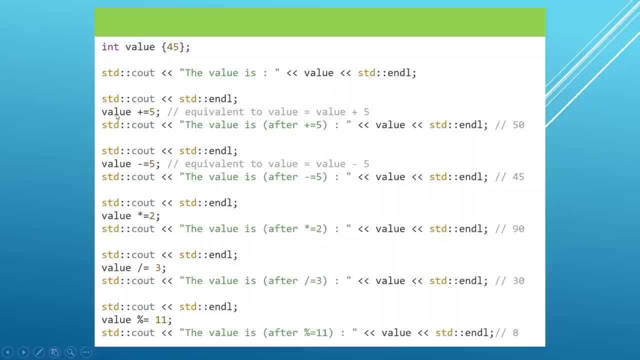 become a 50 and we're going to store that result back in this value variable. here it's going to become 50 and if we print here, we're going to get a 50.. this is the addition version of the compound assignment operator. we also have a version for subtraction and we have an example of that here. 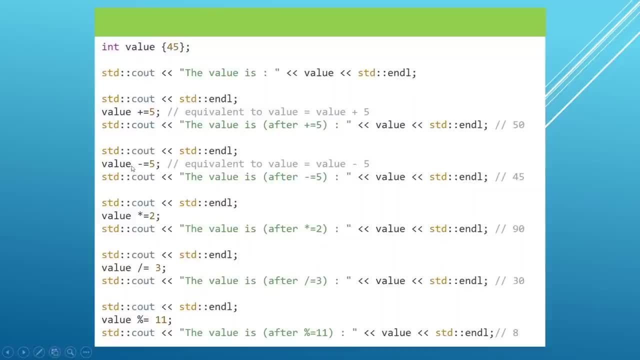 so it's going to take whatever value is in this value variable, it is going to find in a 50.. we're going to subtract 5, we're going to get a 45 and that's what we're going to store in this value here and by the time we hit this std. 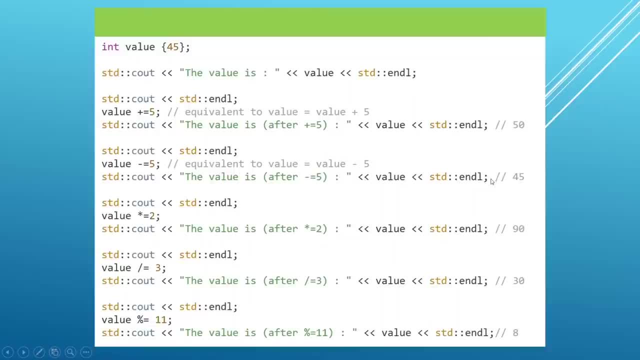 c out statement. we're going to print a 45.. again, we have another version for the multiplication here so that we can really play with all these things. we're going to take whatever value is in here. we're going to multiply that by 2. here we're going to get a 90, and that's what we're going. 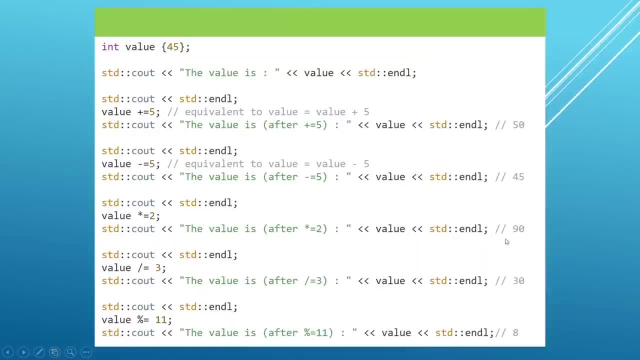 to store back in this value and if we print here, we're going to get a 90 printed out. we're going to go down and do a version for a division. the value is 90, we're going to divide that by 30 and we're going to store the result back in value here and we're going to get a 30. 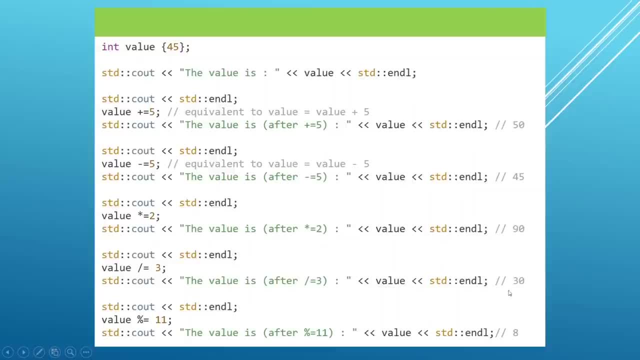 stored in here and if we print out, that's what we're going to get here. we also have a modulus version of this and it works really well. here we have in a 30. we're going to take it and do modulus 11. and what is the reminder of dividing 30? 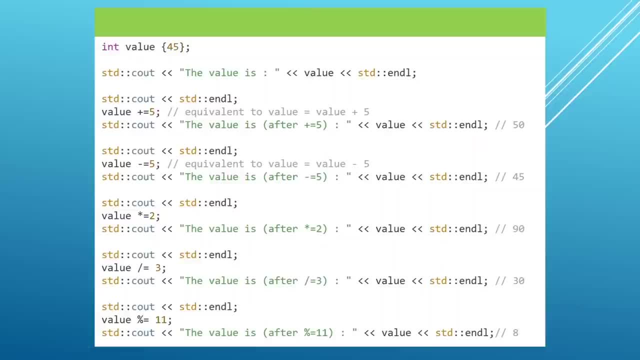 by 11.. the reminder is going to be 8, because 11 can only fit in 30 two times and we're going to be left with an 8, because 30 minus 22 is 8 and that's what we're going to store in the value here. 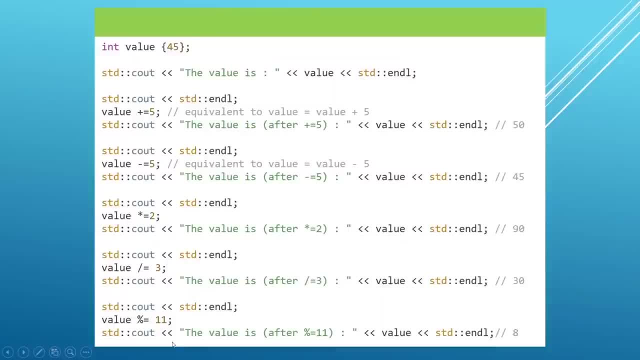 and if we print out, that's what we're going to get again. if you have trouble understanding this modulus operator here, please go back in a few lectures back. we had a chance to learn about it. make sure you understand it and then come back here and this is all going to make sense. this is really all compound. 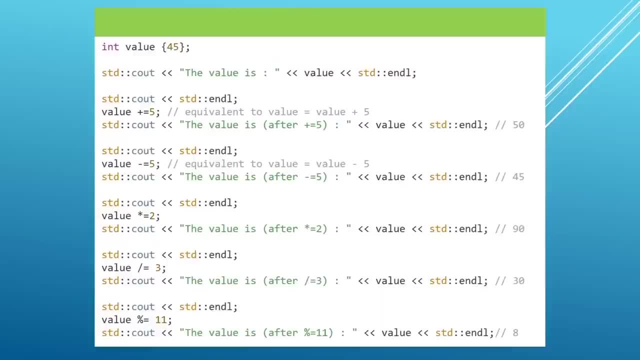 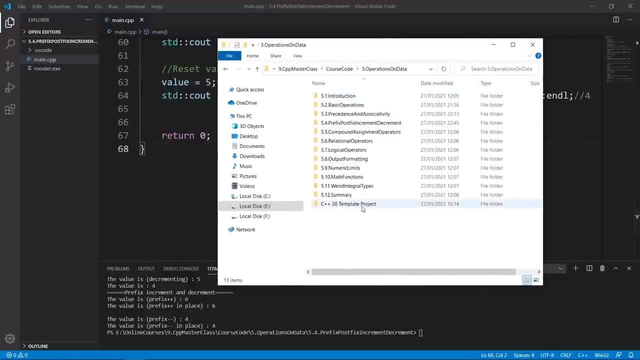 assignment is all about. we're going to head to visual studio code and actually play with us. okay, here we are in our working directory. we're going to copy our template project, as we always do, and we're going to put that in our compound assignment operators. lecture here. 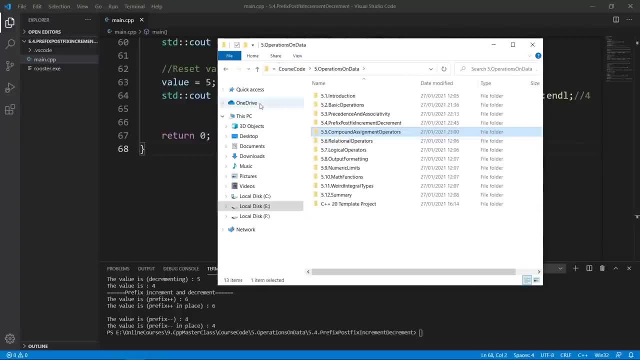 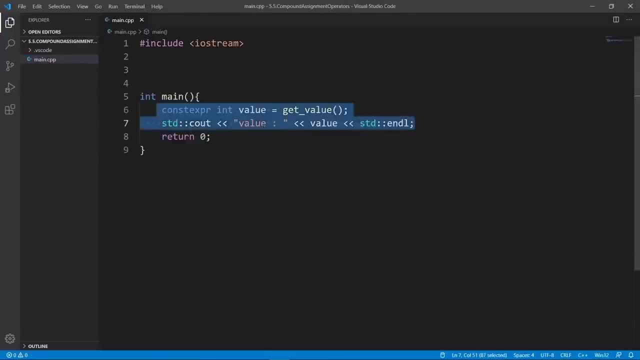 we're going to come up and we are going to open this folder in visual studio code. the project is going to show up in here and we're going to open our main cpp file and we are going to remove what we don't need. we are going to put in our code so that we can start exploring this. we have a 45 in this variable. 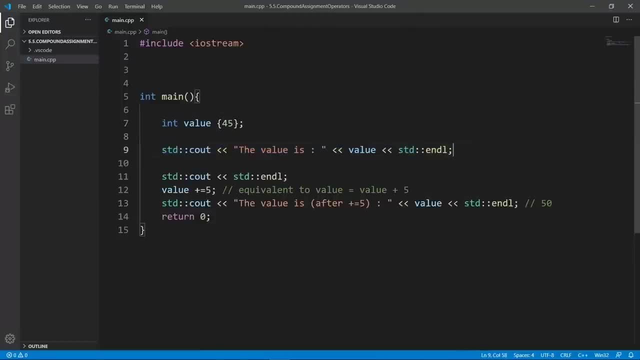 here, which is an integer. if we print it out, we're going to get a 45, and down here we are doing a compound addition. so what we are doing here, we're going to grab whatever value is in this variable. we're going to add a 5, we're going to get a 50 and that's what is going to be stored in here. 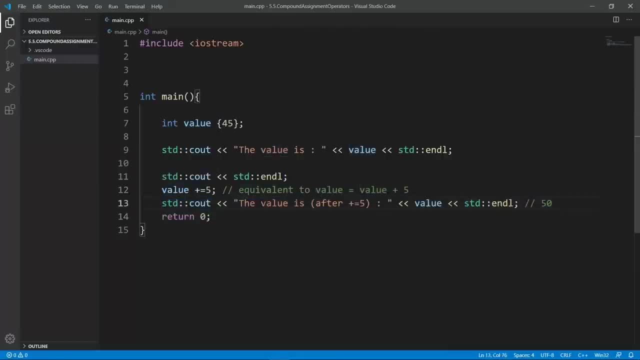 and if we print this out, we're going to get a 50- let's put in a terminal here so that we can see this running. and we're going to run the task to build with gcc, as we always do here, and if we run, our rooster executable. 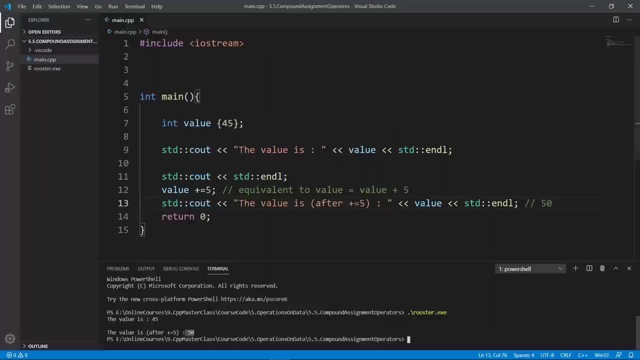 we're going to get. the value is 50 and that's what we expect here. okay, this is the addition version of our compound assignment operator, and it is really equivalent to doing this in two steps. saying value equals value plus 5. you're going to get the same result if you do that here. actually. 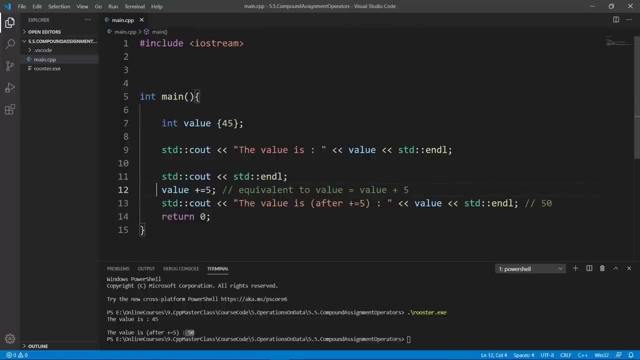 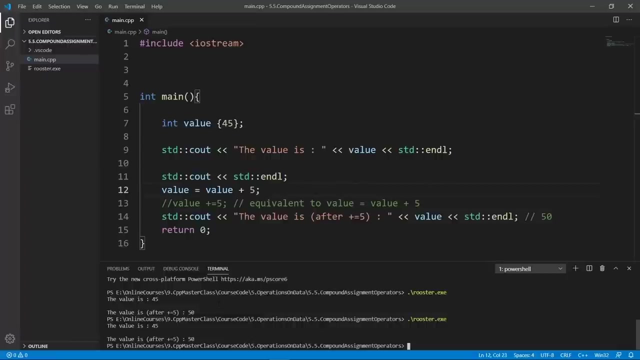 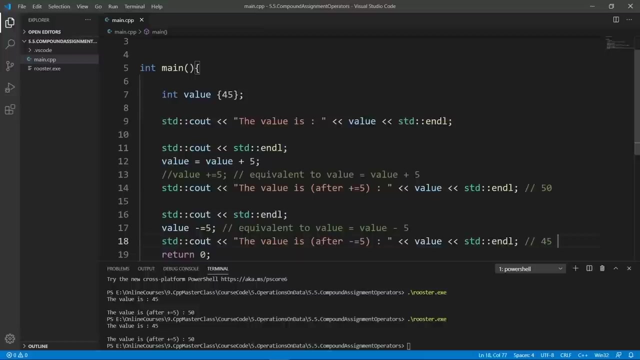 let's do this so that you don't think that i am making this up. so let's comment this out. and we are going to say: value equals value plus 5, and if we build again, run the gcc task and run the application, we're going to see the same thing. we can also go down and run the subtraction version of this. 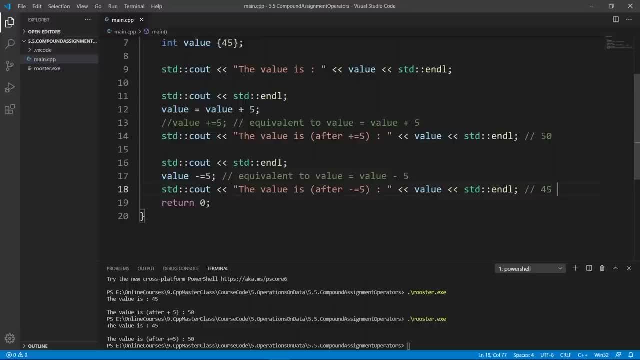 example here. here we are taking the value that we have in here, which is a 50. we are subtracting 5, we're going to get a 45, and a 45 is what we're going to store in this value here. that's what we're going to see if we print this out. so 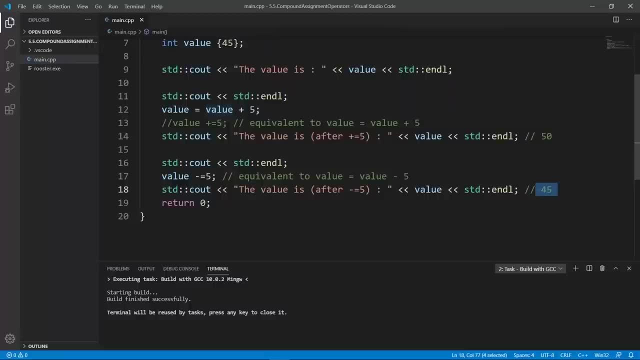 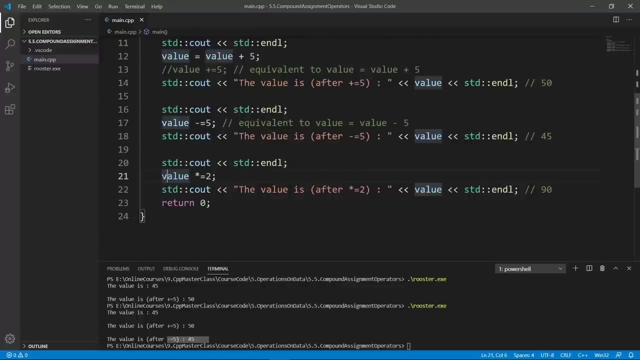 let's run the task to build with gcc so that our changes are reflected in our output. we're going to run this and we're going to get a 45. this is what we expect. we are going to go down and do a multiplication version of this. here we have our compound assignment statement. 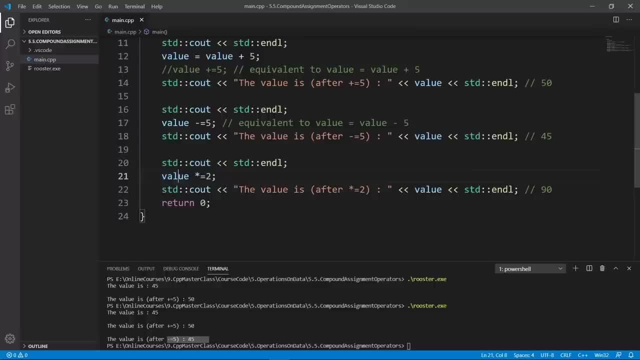 we are taking whatever value we have in here, which is a 45, we're going to multiply that by a two and the result of that is going to be 90 and we're going to store that back in value here and if we print value here, we're going to get a 90.. let's weld this, run the gcc task and we're 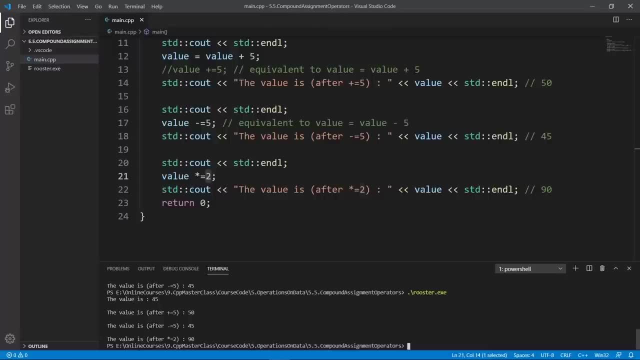 going to run our program and we're going to see that we're going to see this 90 here. we can go down by a few lines and put in the code to play with a division version of this again. this is going to do really the same thing, only it's going to be doing this for division we're going to take. 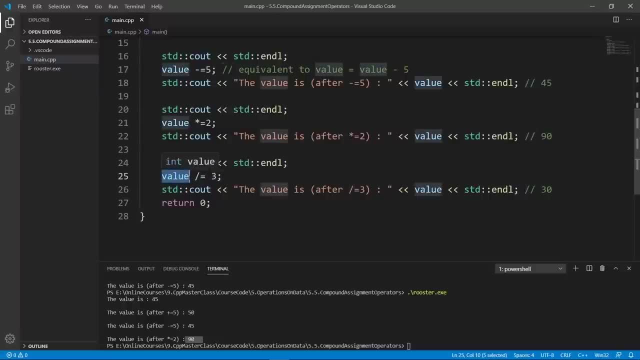 whatever value we have in here, which is going to be a 90, we're going to divide that by 3, we're going to get a 30, and that 30 result is going to be stored back in value here and if we print this out, that's what we're going to get. let's build again, and the build is going to go through if 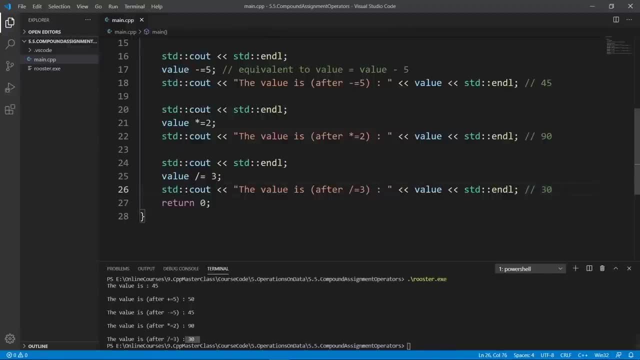 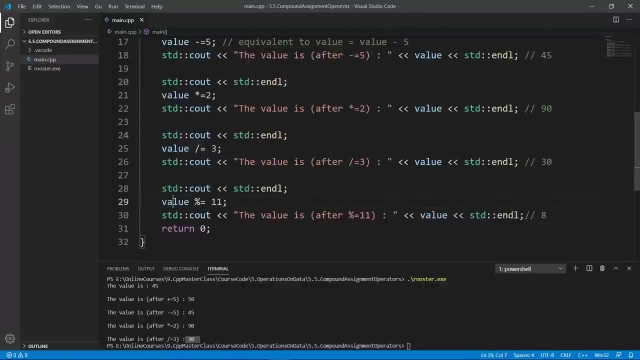 we run our program. we're going to get a 30.. we are going to go down by a few lines and put in a modulus version of this. we're going to grab whatever value we have in this variable here, which is going to be 30.. we're going to do modulus 11. 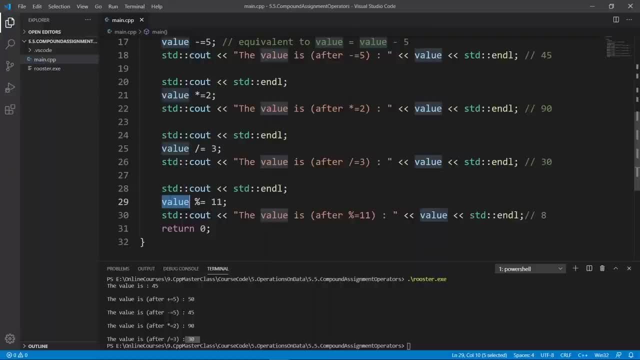 on that value and that's going to be basically 30 modulus 11.. the result of that is going to be 8 and we're going to store that result in value here and if we print that out, that's what we're going to see in this output statement. here we can build again, run with gcc, and if we run our rooster, 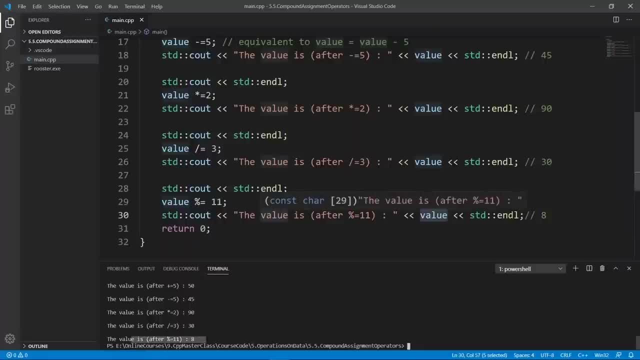 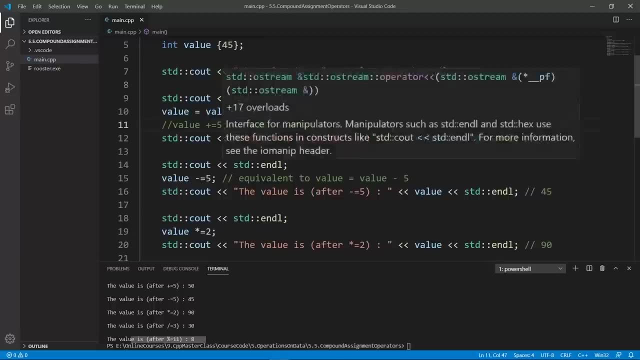 we're going to get an 8 printed out, and this is really all these compound assignments are about. and you might be asking: why go through the trouble to do something like this if i can do this like this? well, c plus plus gives you different way to do things. different people have different 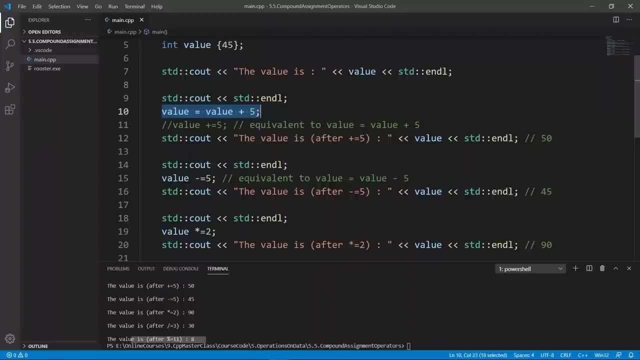 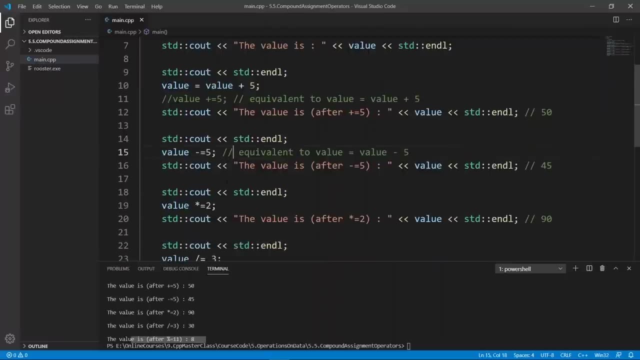 preferences and some people, me included, like to do things this way because it is compact and once you use this, you're going to get used to this. you're not even going to think about it in this lecture here. i just wanted you to be aware of this possibility. 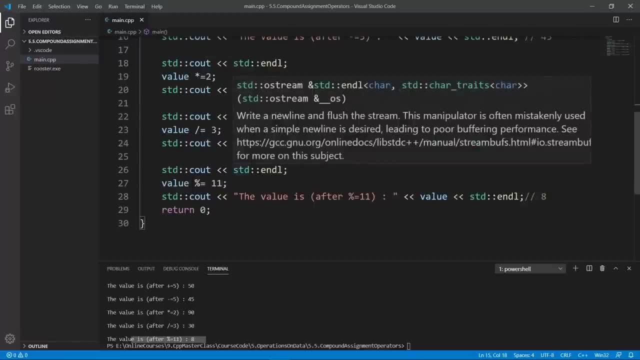 because you are definitely going to see it in c plus plus code out there. this is really all we set out to do in this lecture. i hope you found it interesting. we are going to stop here in this lecture. in the next one we're going to learn about relational operators in c plus plus in. 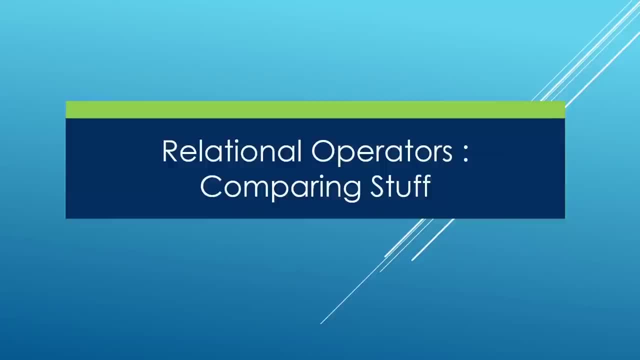 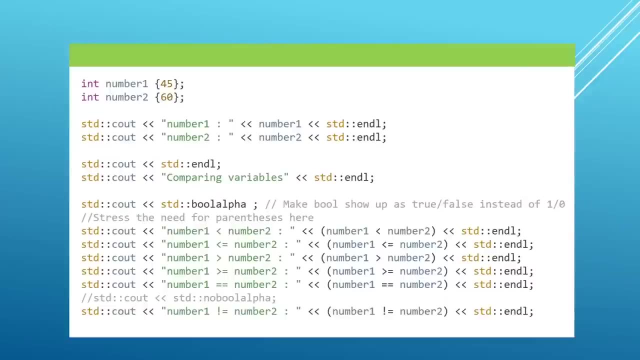 this lecture we're going to learn about relational operators in c plus plus, and these are basically operators you use to compare stuff. let's look at a piece of code here we have two numbers. one is 45 and another is 60. they are stored in integer variables. number one and number two we can print. 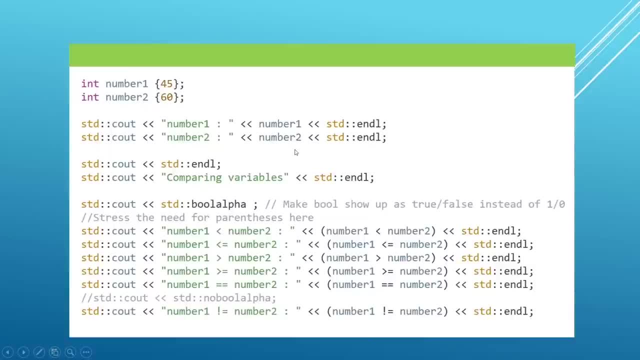 them out and we're going to see them on the console or our terminal and if we go down we can really compare them. we can use the less than operator, less than or equal operator, greater than greater or equal operator. we can check and see if two numbers are equal by using two equal signs. 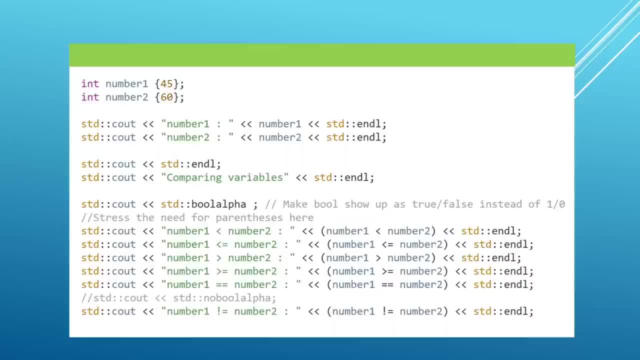 here: be careful about these two equal signs, because if you use one, you're not going to be comparing numbers, you're going to be taking the thing on the right and assigning that to the thing on the left. so if you want to compare, you're going to have to type two equal signs. 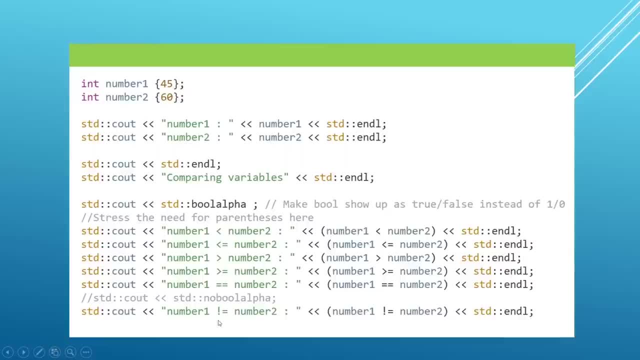 another operator we can use to compare stuff is exclamation mark and equal, which is going to basically test if two numbers are equal and we're going to get the result. one thing you should notice here is that we are wrapping our comparison expression into parentheses. that's because if we don't, we're going to get a weird compiler error that i am. 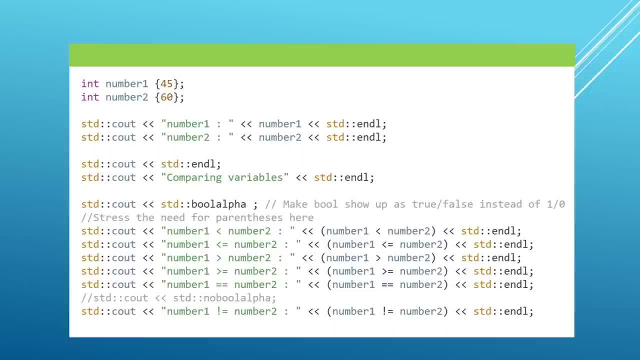 going to show you when we get in visual studio code. but we don't have enough tools to really understand this error at this moment. so what we are going to do is avoid that problem by putting parentheses around our comparison expression. here we're going to go to visual studio code and actually see this in action. here we are in our working. 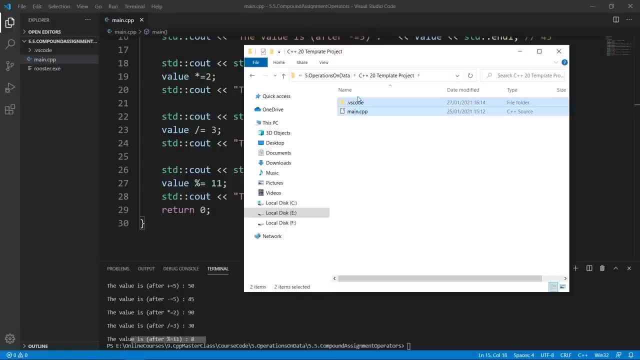 directory. we're going to grab the code from our template here and we're going to put that in the current project, which is relational operators. we're going to go in and put in our code and we are going to open this up in visual studio code. we're going to get rid of. 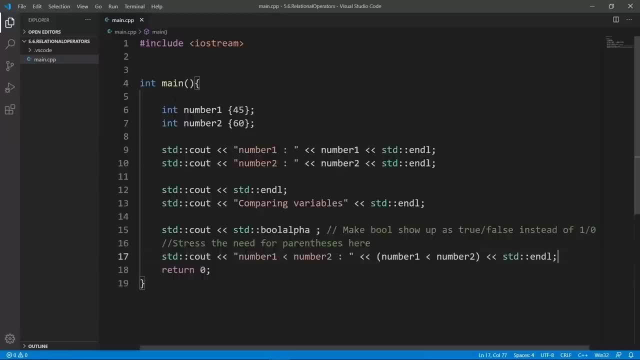 things we don't need here. we are going to put in our code so that we can explore these things. we have two variables. in one we have a 45, in another we have a 60 and these are integers. the name for these variables are number one and number two. we're going to print them out. 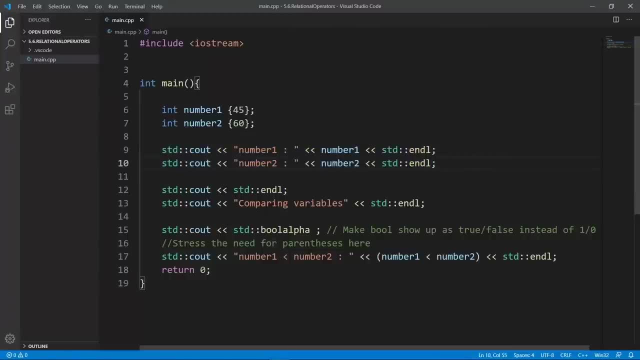 and we're going to see them on the console. now we are going to compare them. one thing i haven't told you yet is that these comparison operators evaluate to booleans. in other words, they are going to return true or false if you look down here. we want to know. 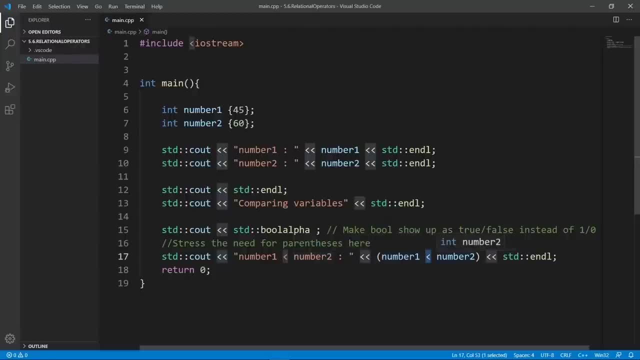 if number one is less than number two and the result of that is whether that's true or false, and this really makes sense. so because of that, we are using std bull alpha here to force stdc out to print this boolean value here as a true or false instead of a one or a zero, and we have seen this. 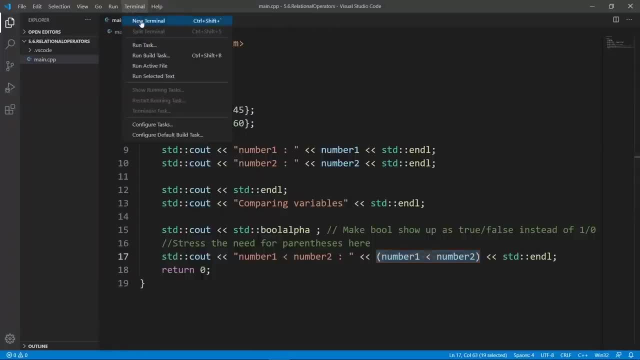 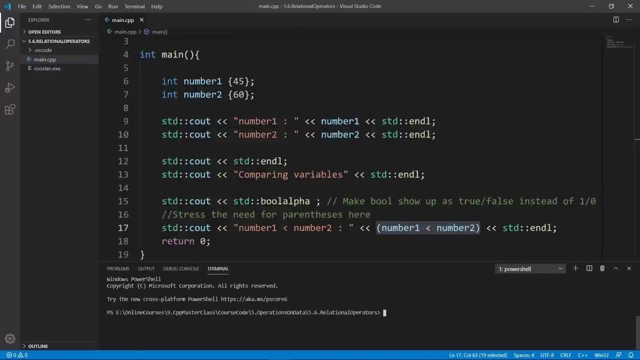 so if we try to build this and run this, let's bring up a terminal we can use and we're going to run the task to build with gcc. if we go down here and run our rooster program, we're going to get our two numbers, 45 and 6, and we want to know if number one is less than number two, and that's. 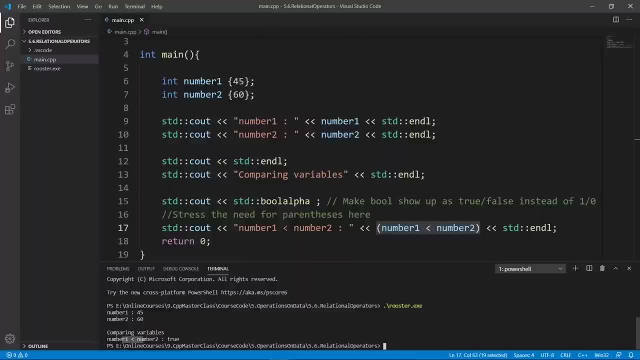 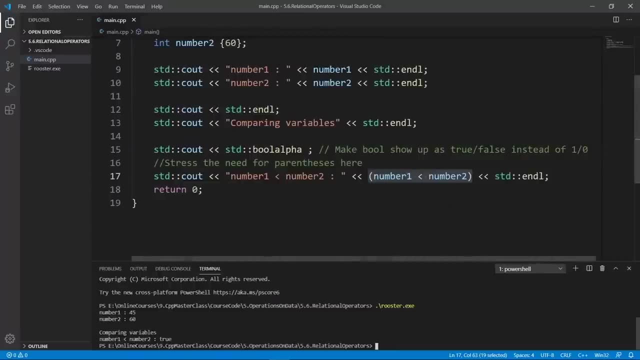 true. 45 is less than 60, so the result of this expression is going to be true. now you know how. one thing i want you to see is what could happen if you didn't use this parenthesis around this expression here. let's try this out. we're going to remove this parenthesis and we're going to try and. 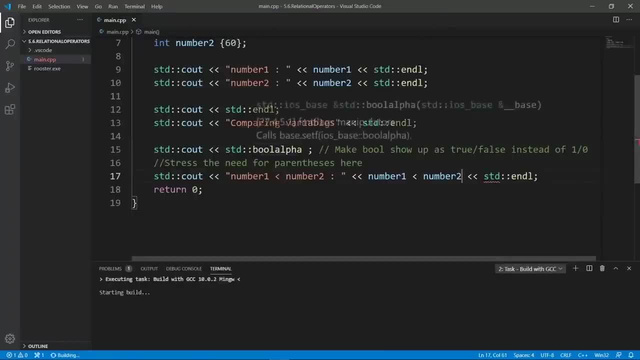 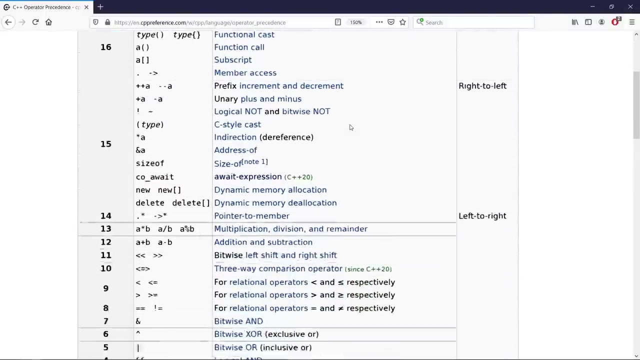 world. we're going to run the task to world with gcc and we're going to get a really weird error because the compiler is going to try and evaluate this operator first. if we go back to our c plus plus operator precedence table and look at the operators we are trying to use in the std cout statement. 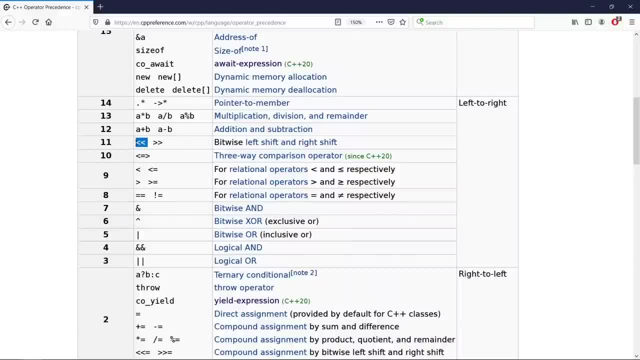 we're going to see that the operator to print fence on the console has high precedence than our comparison operators here. so the precedence for our operator to print fence to std out is 11, so it is higher, and the precedence for our comparison operators is nine and eight, so the 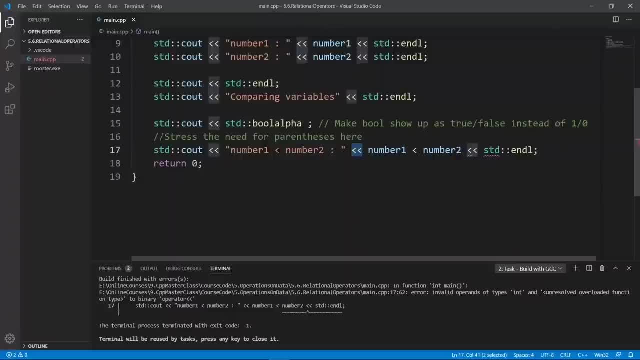 compiler is going to try and do this operator first. if we come back in visual studio code, the compiler is going to try and think that you are printing number one, but then again it's going to see this less than sign and things are going to blow up. we don't really have enough tools to 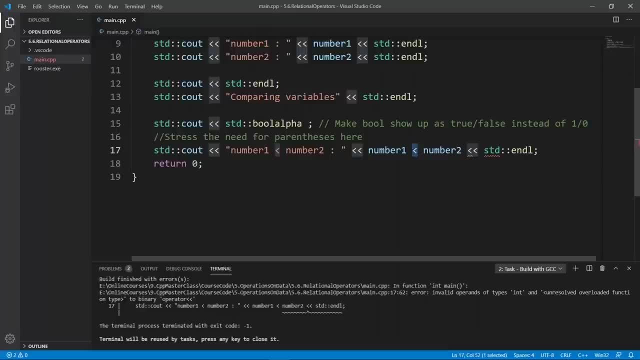 understand what is going on right now, but i just don't want you to see this arrow and show you a way to go around it and move on with your life by comparing stuff in your c++ programs. if you put parentheses around here, the problem is going to go away. let's try and build. 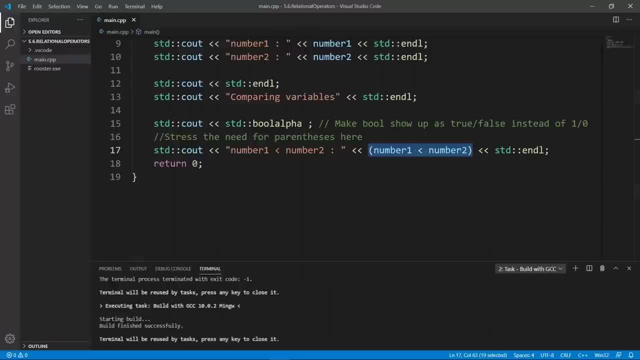 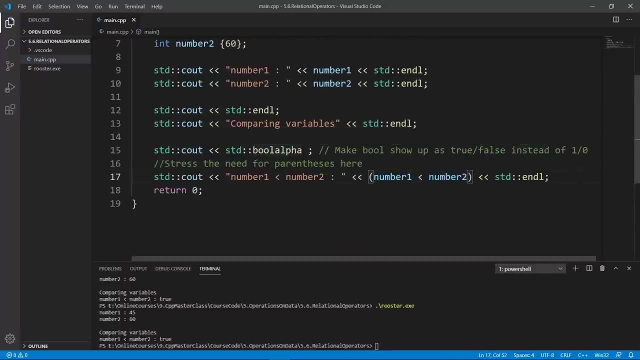 again. we're going to build with gcc and everything is going to go back to normal and we're going to see our output if we run our rooster program here. this is how you can do this. okay, now that we have a basic understanding of this, we can try the other operators, and it is going to be a walk in the park. we are going to go down. 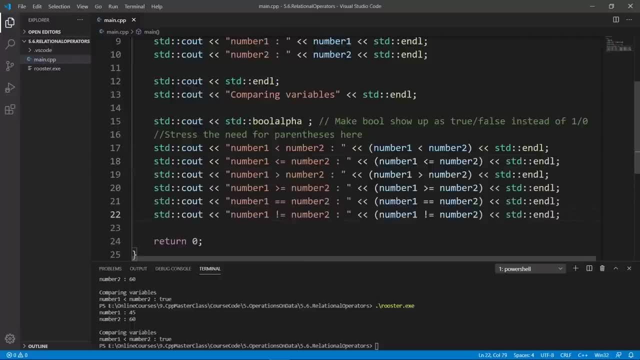 here and put in our remaining operators. we can use less or equal operator to test and see if number one is less or equal to number two. we can use the greater than operator to test and see if number one is greater than number two. we can use the greater or equal operator. we can use the equal. 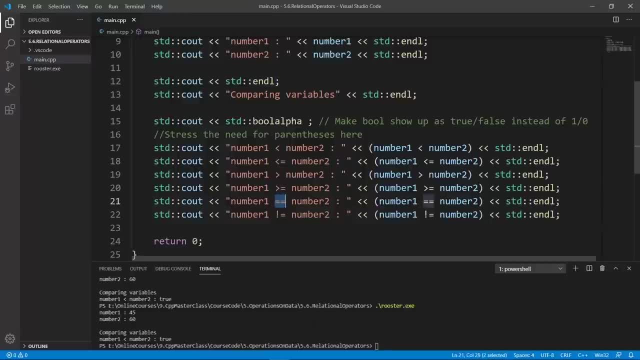 equal operator to test and see if number one is greater than number two. we can use the greater or equal operator to test that number one is equal to number two. and we can use this operator here, which is made up of the exclamation mark and an equal sign, to test and see if two numbers are not. 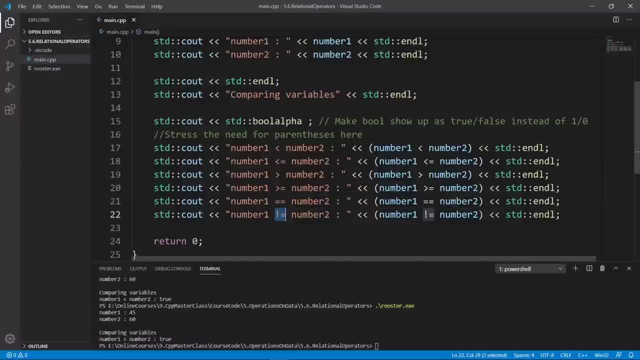 equal and all these operators are going to evaluate to a boolean, basically saying if what you are testing for is true or false. and we can print this out and notice that we have these parentheses around to avoid the problem i just showed you and we can print this out. and we can print this out. 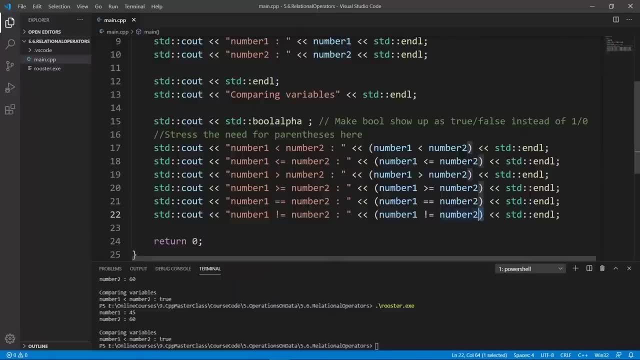 a few minutes earlier and if we run this, we're going to see the results. let's weld this with gcc. as usual, we're going to run our program and you're going to see that number one is less than number two. this is true. number one less or equal to number two: this is also true. number one greater. 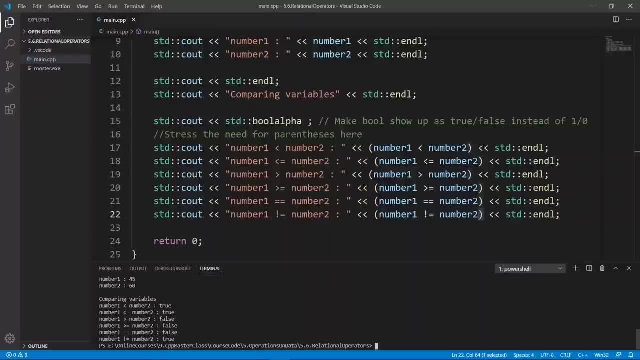 than number two. 45 is not greater than 60, so this is false. it's not greater than equal to, so this is also false. number one equals to number two. this is going to be false. and the last statement that is going to test and see if number one is not equal to number two is going to. 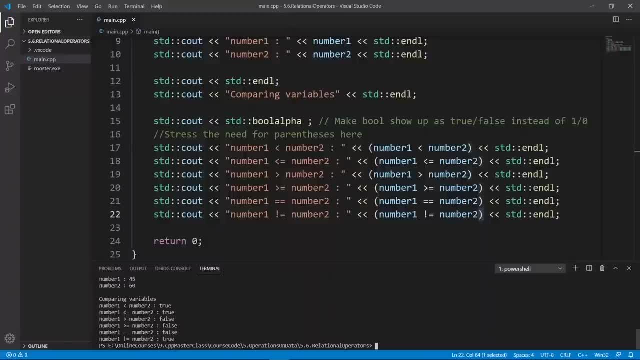 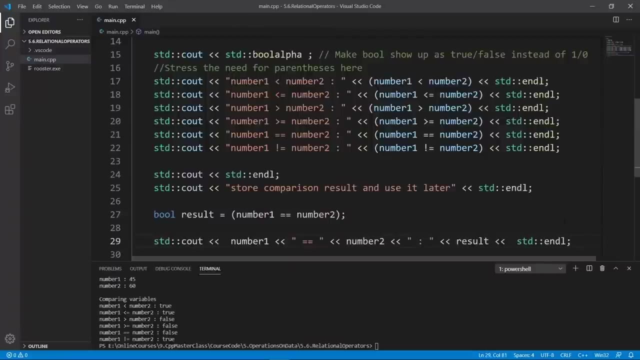 evaluate to true, because number one is not equal to number two. if this is not making sense yet, please go through it a couple of times, and if you have a problem, please do ask me. i will do the best i can to help you out. another thing i want you to see before i let you go is that you can store. 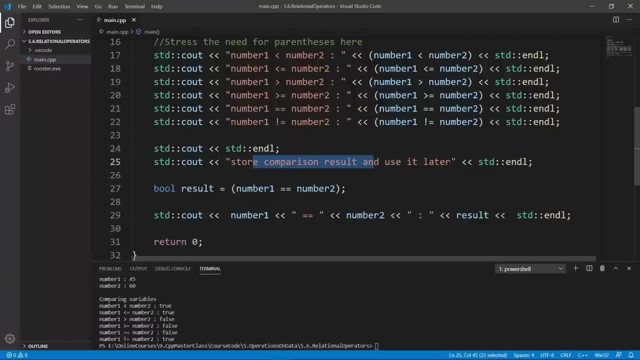 the results of these operators into a variable and use that later in your program. for example, here we can take our expression to compare number one and number two. the result of that is going to be stalled in this bull variable and we can print it out later like this: if we run this, we're going to 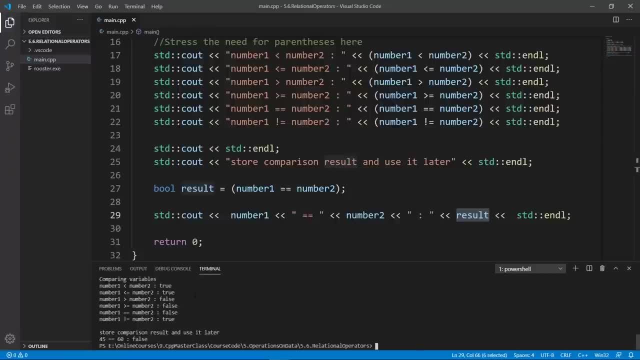 build a virtual16 to do this and we're going to certainly be able to do this in a lot of different projects. but we're going to do this in a lot of different projects and we're going to use this as a with gcc and we're going to run the program. we're going to see that 45 equals to 60 is false and it. 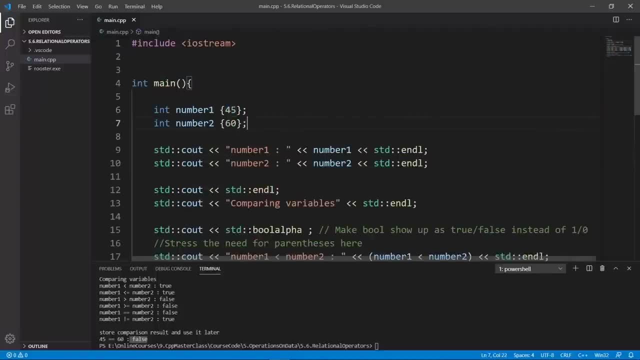 is coming from this statement. here you can try and change these numbers- for example, change this to 20- and see the results that we get, and you can try and run these in your mind and see that they really make sense. if you run rooster now, we're going to get different results because we are now 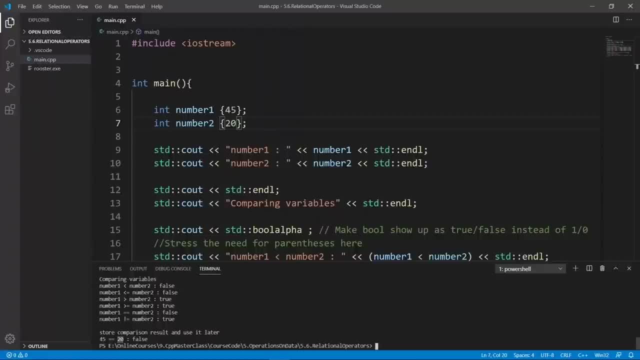 comparing 45 and 20 and here at the last statement, you see that they are not equal. if we put in two equal numbers, we're going to get a true there. let's try this out. we're going to run the task to build with gcc and if we clear so that we get rid of all this noise and run rooster, we're going. 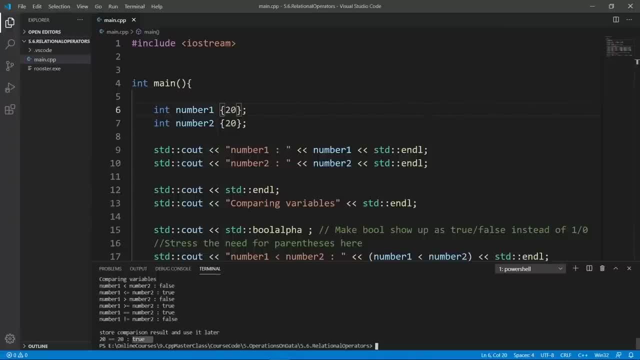 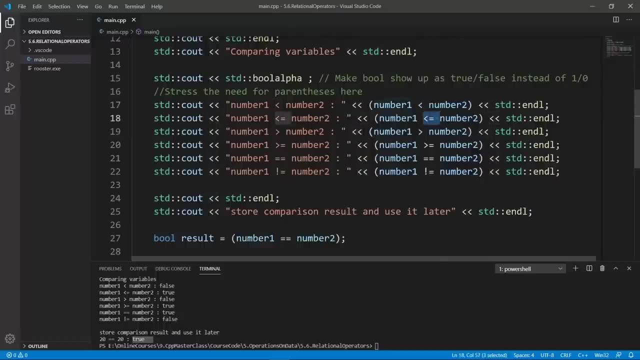 to get 20 is equal to 20 and this is true. this is really all we set out to do in this lecture. i hope you have a better idea of these relational operators in c++. we're going to stop here in this lecture. in the next lecture. 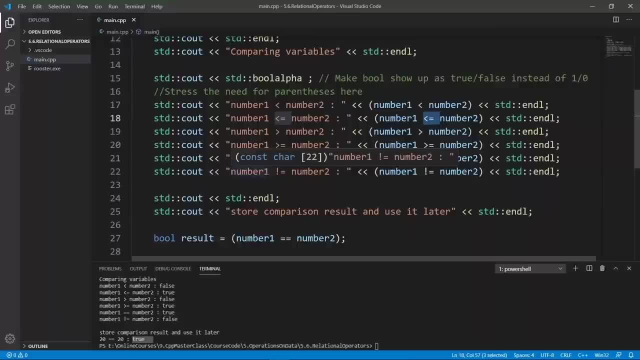 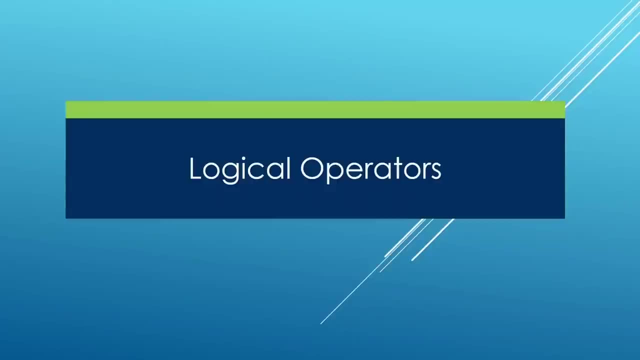 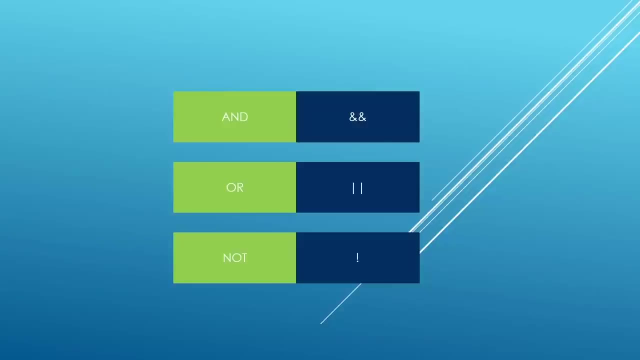 we're going to learn about logical operators in c++. go ahead and finish up here and meet me there. in this lecture we're going to learn about logical operators. these operators will work on boolean operands we're going to look at and first to really make sense of how they work, here is a. 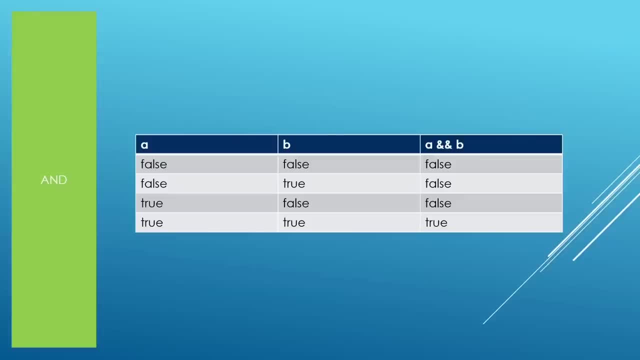 table we can use to try out the and operands operation. it is going to be working on two operands, a and b, and in the third column here we're going to have the result. so if a is false and b is false and we do a and b, the result is: 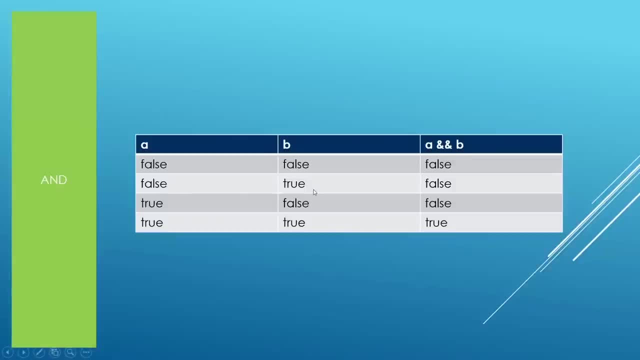 going to be false. if a is false and b is true, the result is going to be false. if a is true and b is false, the result is going to be false. if a is true and b is true, the result is going to be true. the way you can think about this and operator is that if any of the operands is false, 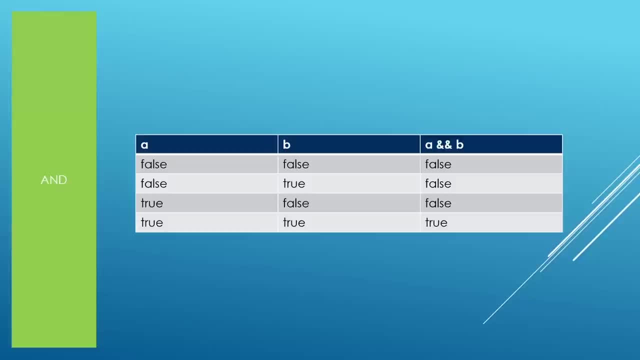 the result is going to be false, and if you really use this way of understanding this, it is going to be really easy. in the first line here we have a false, so the result is going to be false. in the second line, we have a force: it's going to be forced. in the third line, we have a false: the 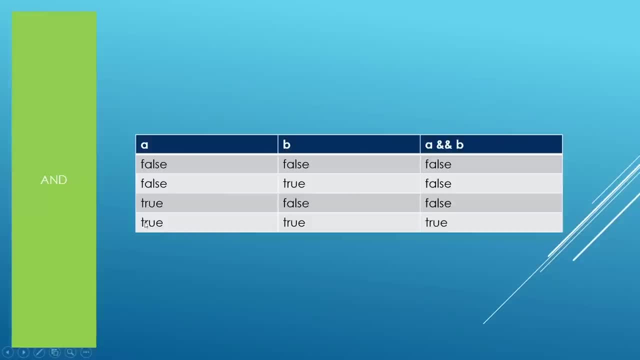 result is going to be false. but in the line number four, here we have a false and we're going to have a false. here we don't have a false. a is true and b is true, so the result is going to be true. another operator we have is or, and it is going to evaluate to true if any of the operands is true. 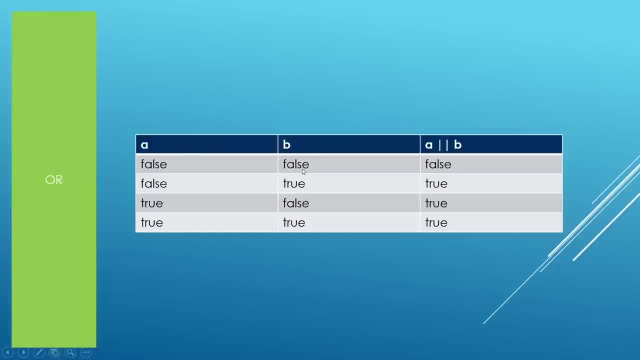 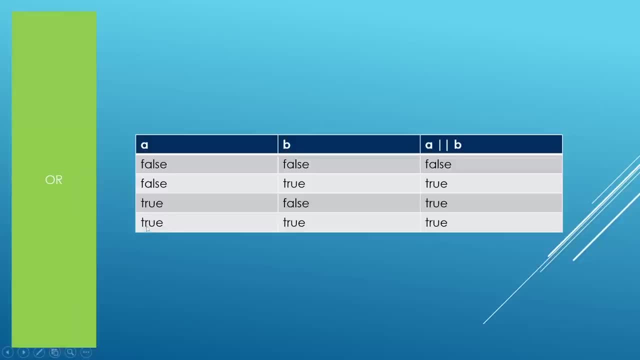 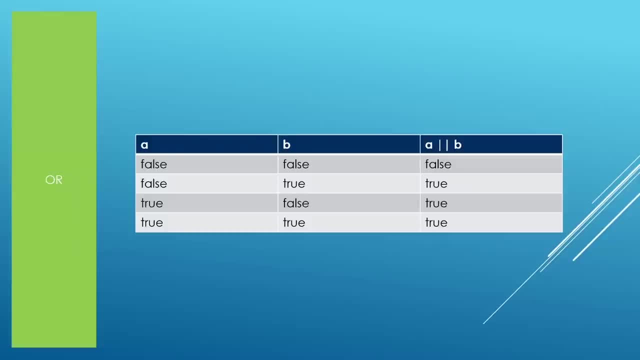 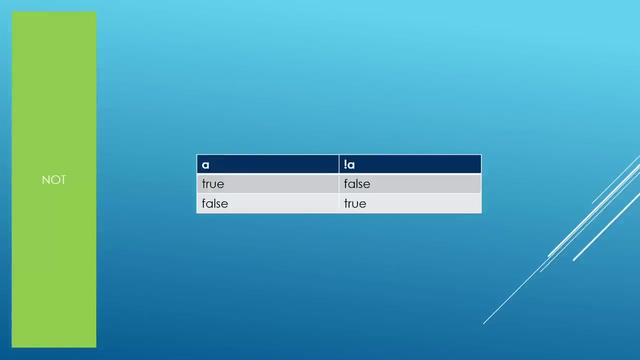 long enough. these things are going to be drilled in your memory. if you have any problem with these operators, just look up tables like this and you can find whatever it is you need without really memorizing these things. another operator is the not operator, which is going to negate whatever you. 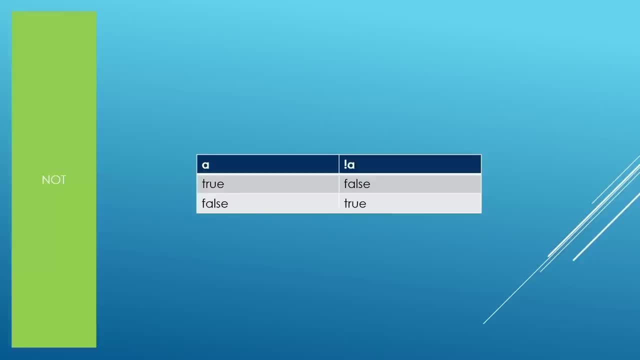 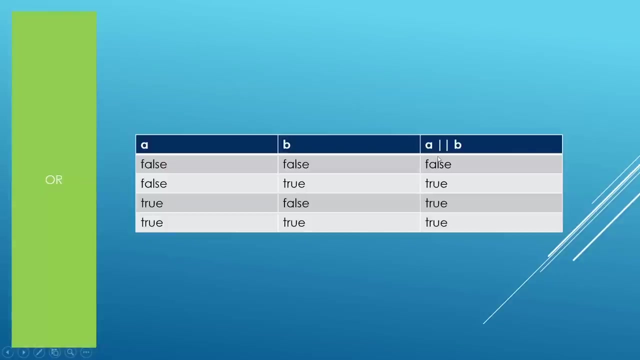 gave it. so if a is true- and when you get to that, we're going to get a false. if a is false, and when you get to that, we're going to get it true, and we use this exclamation mark to say that we are negating something. if you go back to, or it is denoted by these two vertical bars and the end. 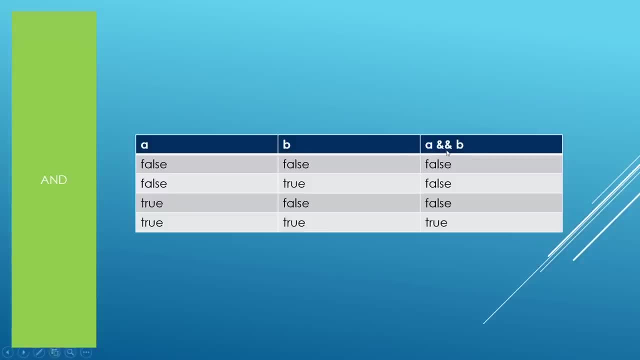 operator is denoted by these two ampersand symbols here. okay, now that we know about these logical tables for this logical operation, we are going to go back to the first line and we are going to go back to the first line and we are going to go back to the first line and we are going to go back to the first line. 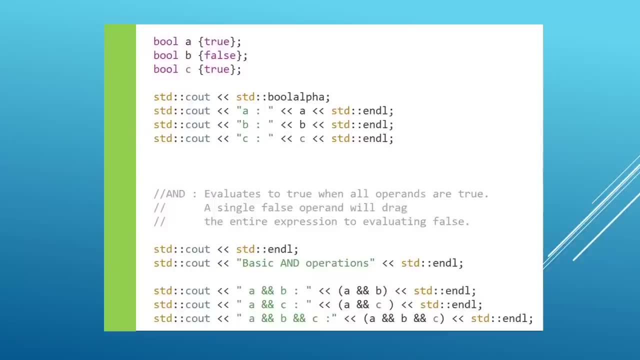 we can actually try to use them in code here. we have three boolean variables. we have a, b, c. a is true, b is false, c is true. we can print them out and you see that we are setting up sddc out to give us the results in the format of true and false instead of ones and zeros. 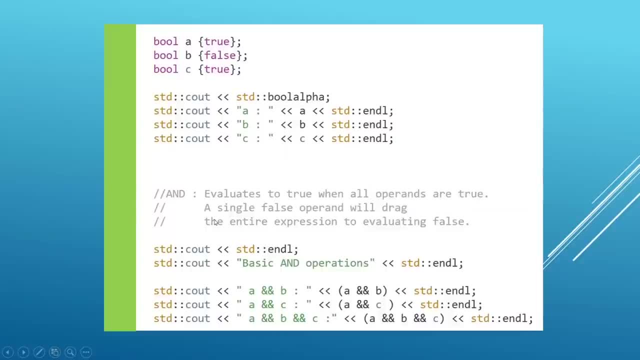 and down here you see that we are trying to use the and logical operator. down here you have a and b, a and c and we are doing this on three operators and chaining these things up. so we are saying a and b and c and let's try and do this in our mind to see that we really understand this. we have seen. 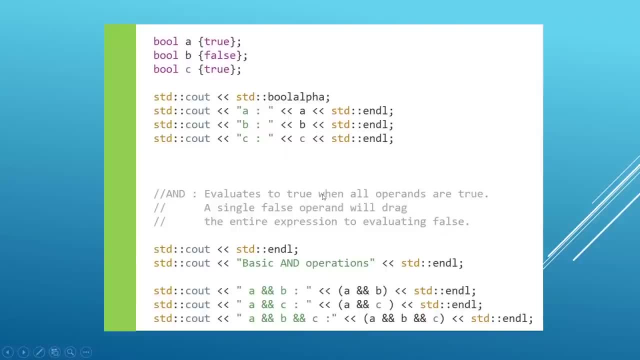 that the end operator evaluates to true when all operands are true. another way to say this is: the end operator evaluates to false if any of the operands is false. so we're going to add a and b. a is true, b is false, so the result is going to be false because we have a false in here. a and c is. 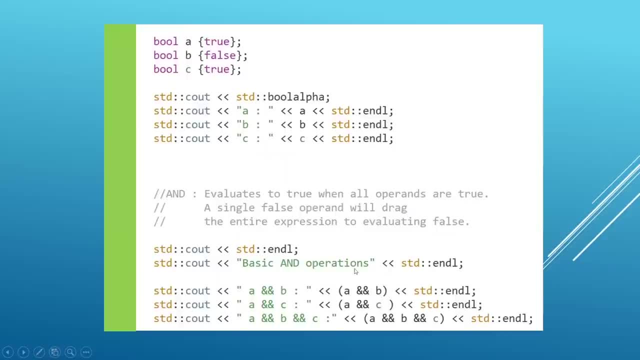 going to evaluate to true because a and c are true. a and b and c is going to evaluate to false because we have a false in here. even if you have 1 000 truths and you end that with one false, that's going to be dragged down to evaluate to false. that's what we are seeing here. we can also do. 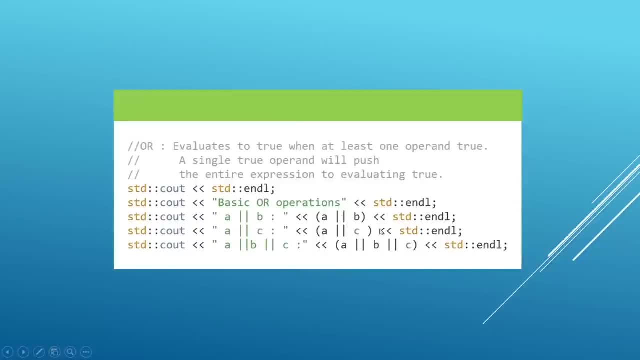 or operations on these things, and this is going to give you a true. if any of the operands is true, we know that a is true and b is false, so this is going to evaluate the true. a and c is also going to evaluate to true because a is true. a and b and c is going to evaluate the true because a is true. 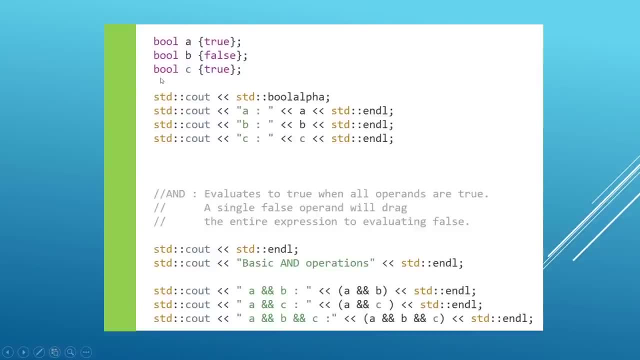 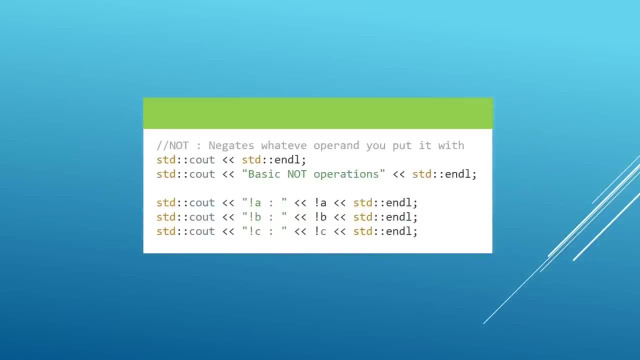 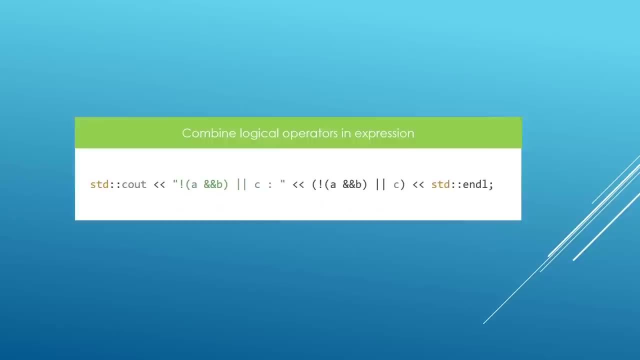 so let's go back and see this. these are the values we're going to be using here. we can also try out the not operator and it is going to negate whatever we give it. so if a is true, we're going to get a false. b is false, we're going to get it true. c is true, we're going to get a false another. 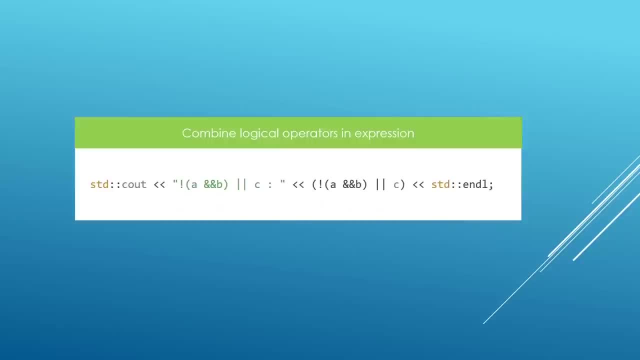 thing you can do is combine these logical operators so we can do something like a and b and all of that with a, c, and you should notice that we are wrapping our expressions here in parentheses so that we don't have the same problem we experienced and explained. 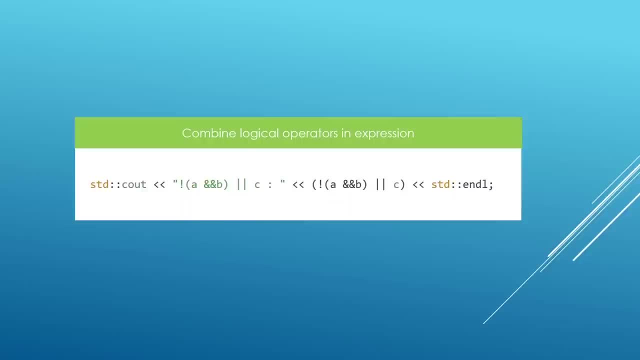 in the last lecture, and one thing you should know is that for the compiler to evaluate these things, we are going to follow the rules in our table for precedence and associativity, but we used parentheses to really make this easy to follow. so we are going to end a and b and the result 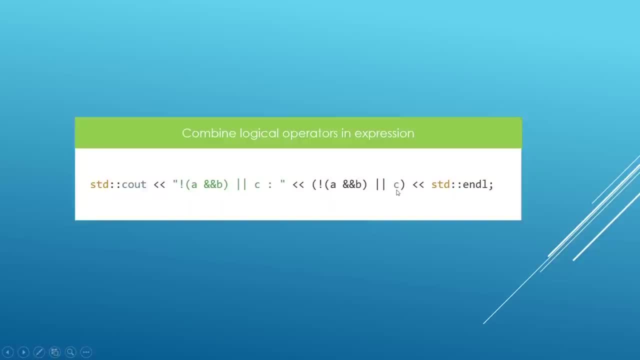 of that is going to be ordered with c and you can try and do this in your mind and you're going to figure this out. but we're also going to go to visual studio code in a minute and we're going to see all these things in action. the last thing you can do is combine logical and relational. 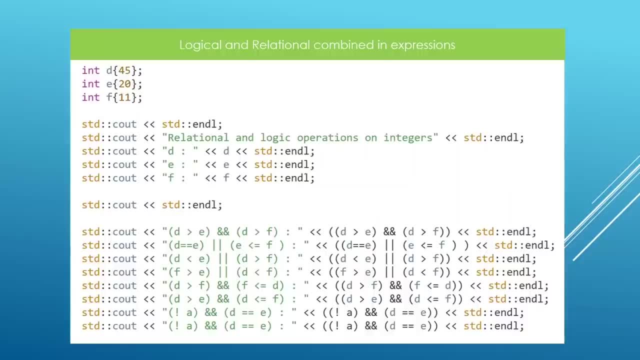 operators into expressions. for example, here we have d, e and f. they are integers and we can print them out like we are doing here, but we can do something like d greater than e and we're going to end the result of that with d greater than f and uh, we know that these relational operators 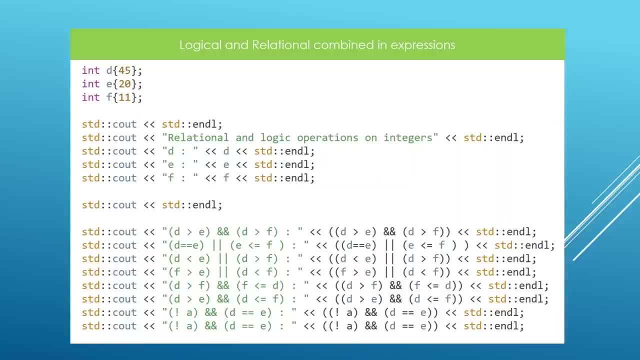 evaluate two booleans so we can use these booleans with logical operators, like we have been doing all along in this lecture. so, for example, let's evaluate the first one here in mind, so that you really see what this is all about. d is 45, e is 20, so d greater than e is going to evaluate to true. 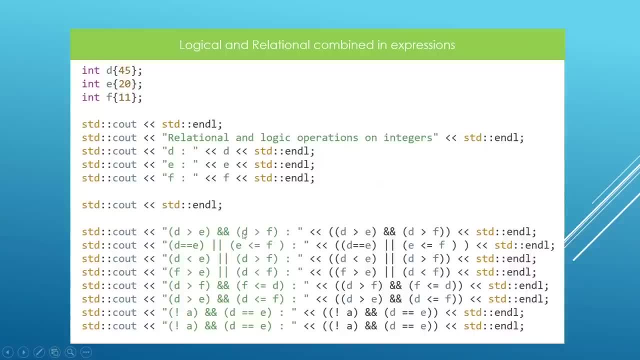 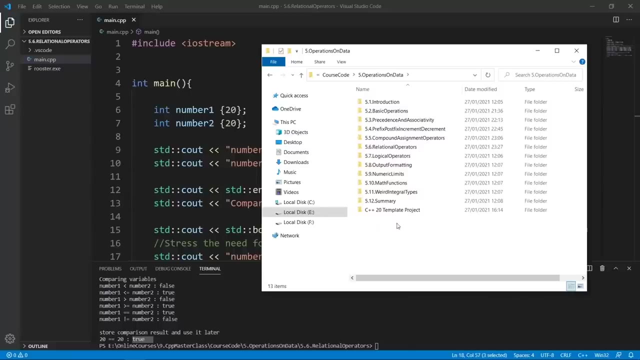 d greater than f. that's also going to evaluate to true. so true and and true. that's going to evaluate to true, and this should print a true on the terminal. we are going to go to visual studio code and actually play with these things. okay, here we are in our working directory, we're going to jump into our template project and copy. 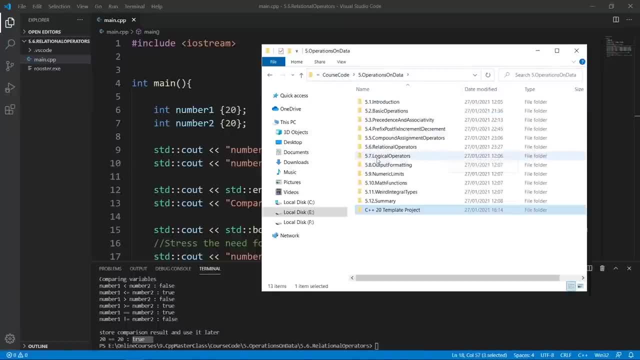 the files we need and we're going to put them in our lecture on logical operators. we're going to put that in here. we're going to open up this folder in visual studio code and it is going to show up here in visual studio code. we're going to get rid of what we don't need and 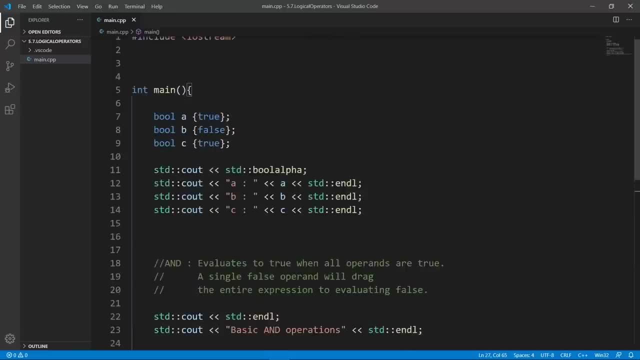 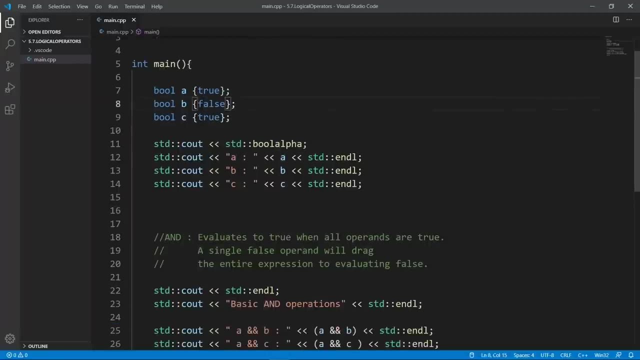 we are going to put in the code to play with these things. we have three boolean variables: a is true, b is false, c is true and we can print them out and we're going to see their values and you see the setup here, so that sdc out is going to show thanks in the format of true and false. 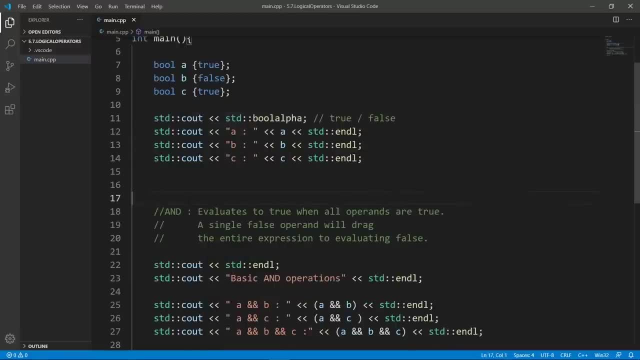 and down here we are ending a few values, so we are going to show things. and down here we are ending a few values, values. so down here we are ending a few values. We are using the AND operator and it is denoted by these two ampersand signs. 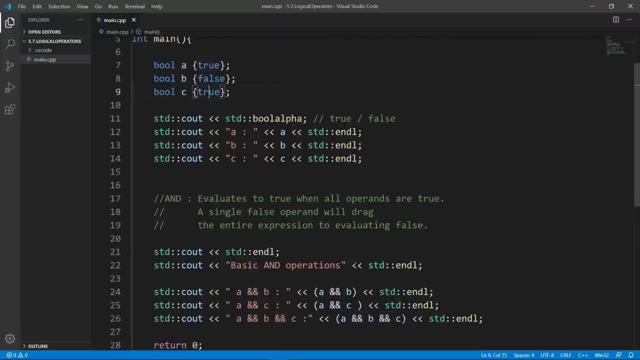 So A is true and B is false and C is true. A and B is going to evaluate to false because we have a false in here And again. if this doesn't make sense, please do consult the tables for all these logical operators. 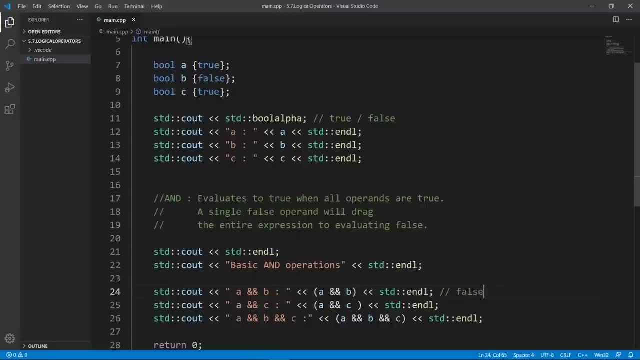 And all these things are going to make sense. This is going to evaluate to false because we have a false in here, And A and C. we have true and true. So this is going to evaluate to true And A and B and C. this is going to evaluate to false because we have a false in here. 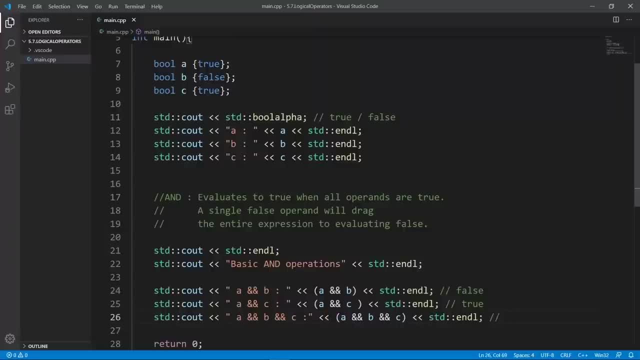 Remember, as soon as you have a false in your AND logical operation, you're going to get a false in your result, So we're going to have a false here. We can try and compile this and see if this is actually what we expect. 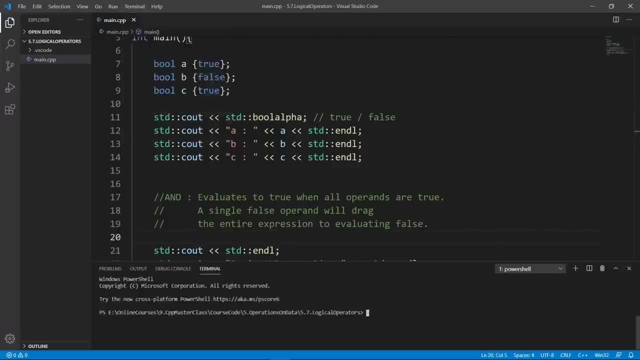 We're going to bring up A terminal we're going to use here And we're going to run the test to build with GCC And if we run our rooster program, we're going to see that A and B is false. This is what we expect. 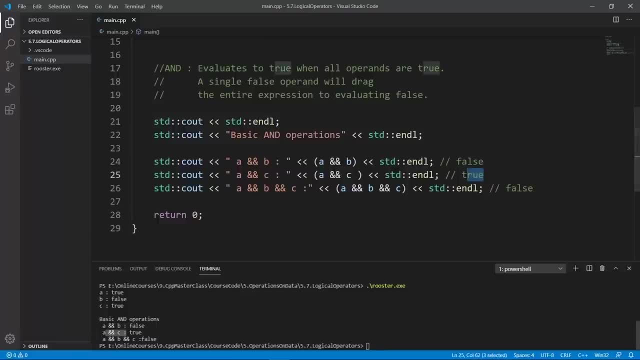 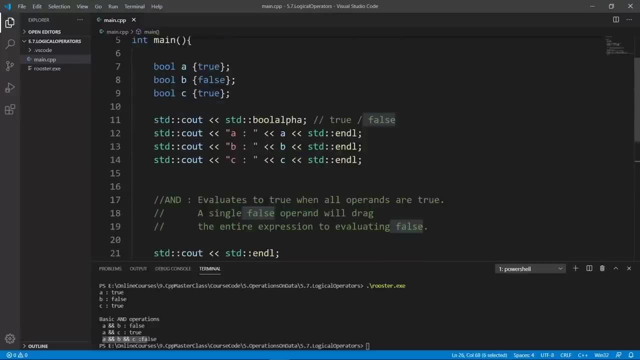 A and C is true. This is what we expect. A and B and C is false, And this is what we expect. This is how you can really play with your AND logical operator. If you want, you can change things up to really. 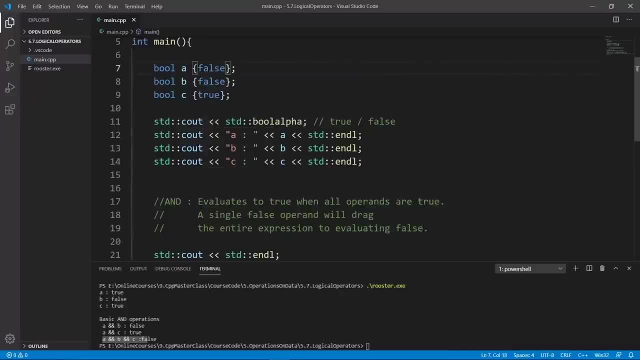 Try and see if they live up to your expectations. Now we have changed A to false. Let's try and build again. We build with GCC and we're going to run our program and we're going to get. A and B is false because they are all false. 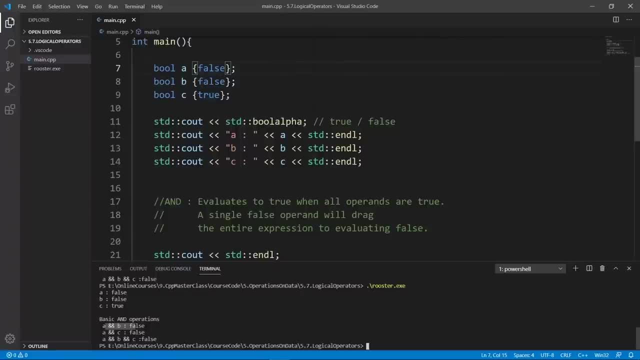 A and B are false, So false, and false evaluates to false. A and C is false because A is false, So we're going to get a false as the result. A and B and C is also going to evaluate to false. OK, we have these things in here. 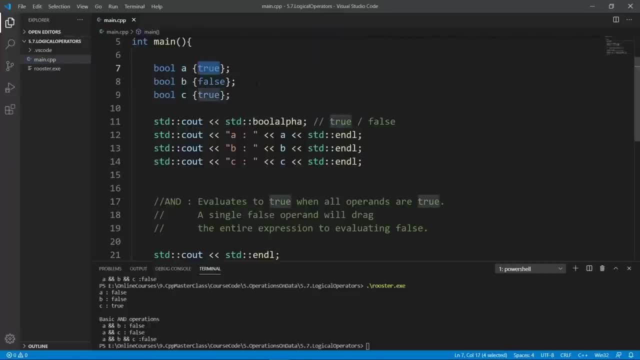 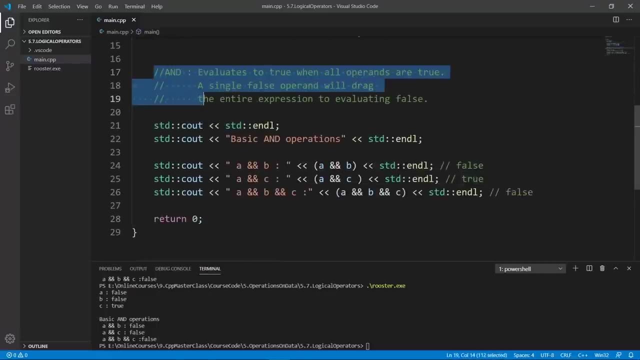 Let's bring this back to what it was before. So A is going to be true, B is going to be false, C is going to be true And we're going to try and play with the OR operator. We are going to go down and put in code to actually play with this. 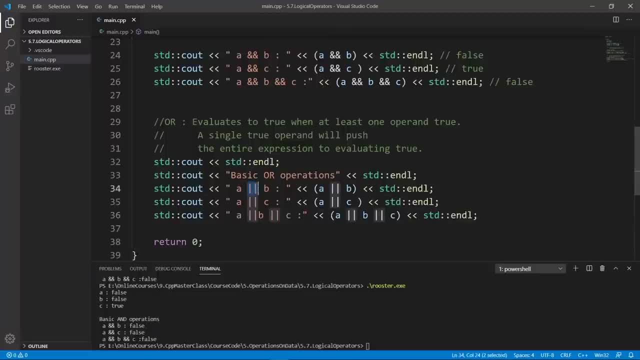 And it is really nothing special. We are just using the OR operator here, which is denoted by these two verticals, These two vertical symbols, and OR is going to evaluate to true when at least one of the operands is true. OK, so we have our values here. 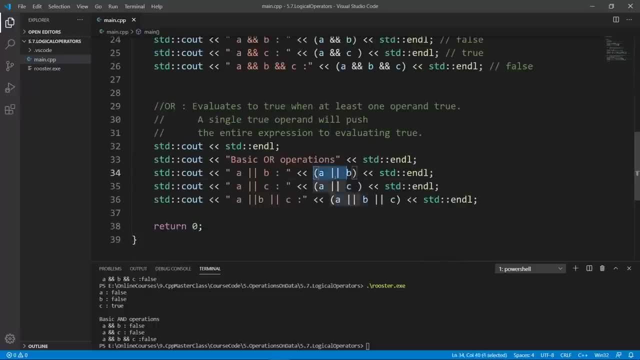 A is true, B is false, C is true. A or B is going to evaluate to true because A is true. A or C is going to evaluate to true because A is true. A or B or C is going to evaluate to true because one of these things is true. 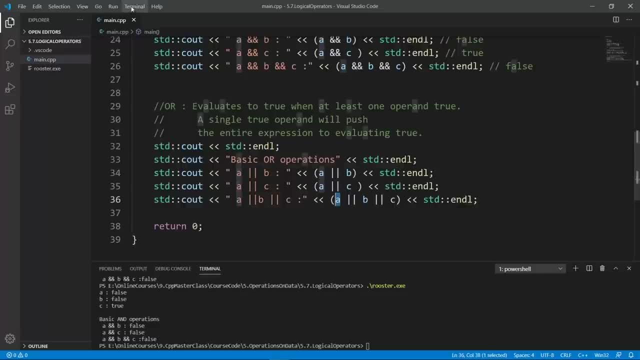 And A is true here. We can try and run this. We're going to build this first with GCC And if we run this, we're going to go down here and run rooster again And you're going to see that all these things are true here, because one of these things is true. 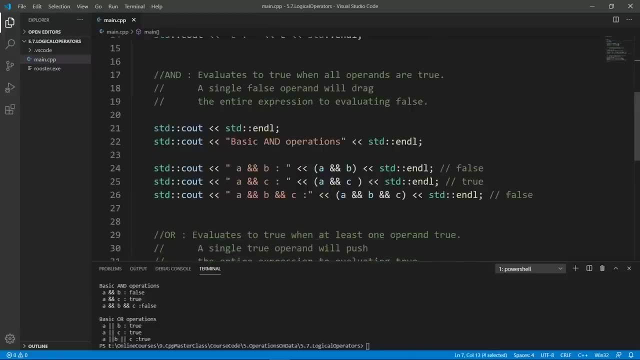 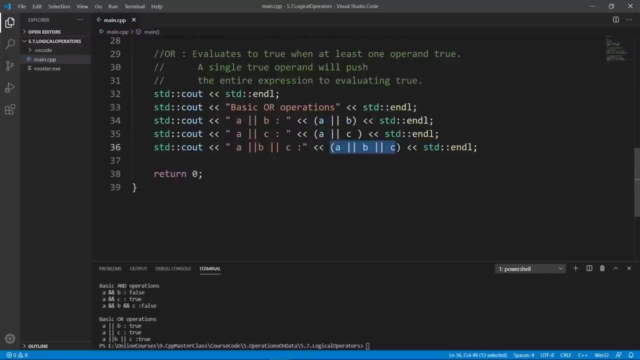 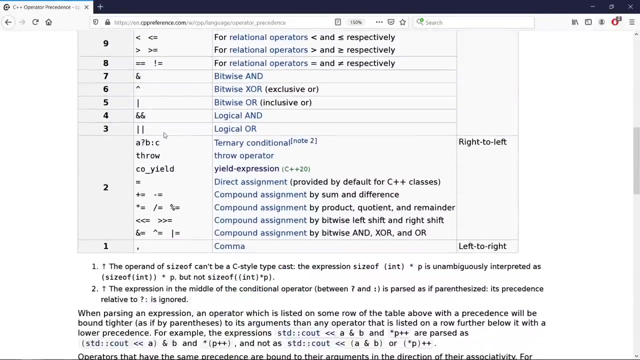 And as long as you have one true operand, your OR operation is going to evaluate to true. And again, this is following the precedence and associativity rules we have. If we go back to our table in our browser, we're going to try and look at logical OR. 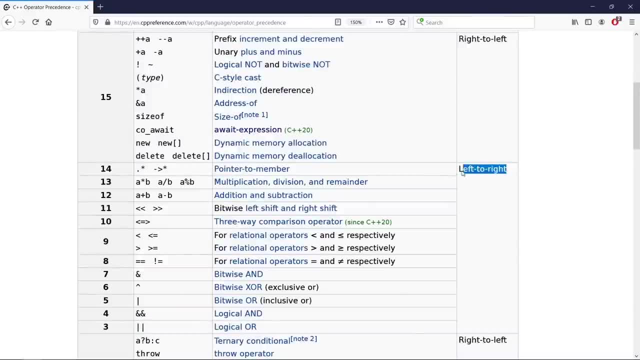 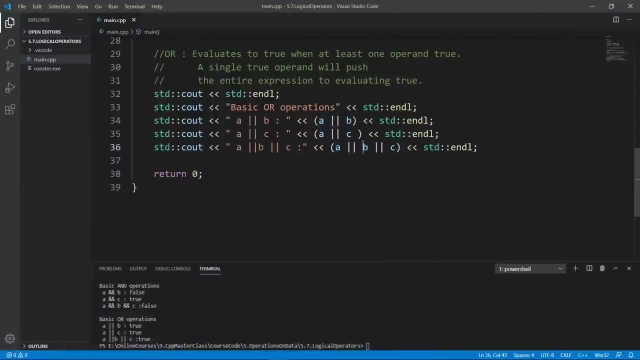 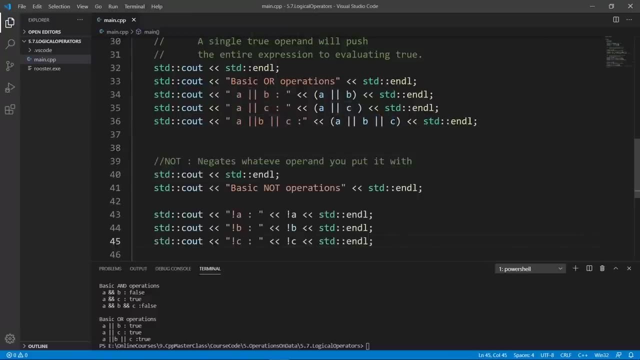 It is left associative. So we're going to try and evaluate this from left to right. So we're going to OR A and B and the result of this is going to be ORed with C. We have also seen the NOT operator, which is denoted by the exclamation mark here. 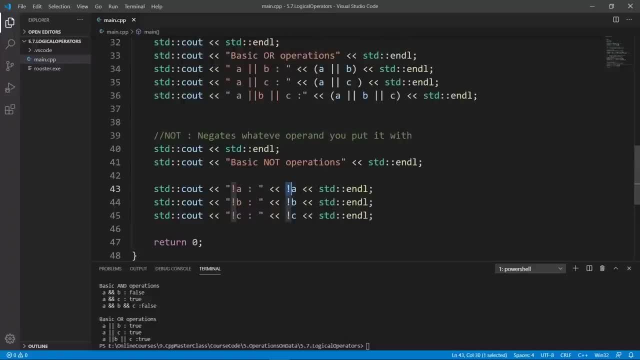 And what it is going to do. It is basically flip off or negate, whatever it is you have. If you have a true in your variable, the result is going to be false. If you have in a false, the result is going to be true. 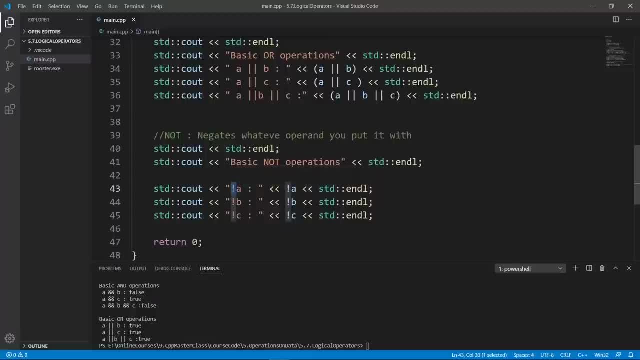 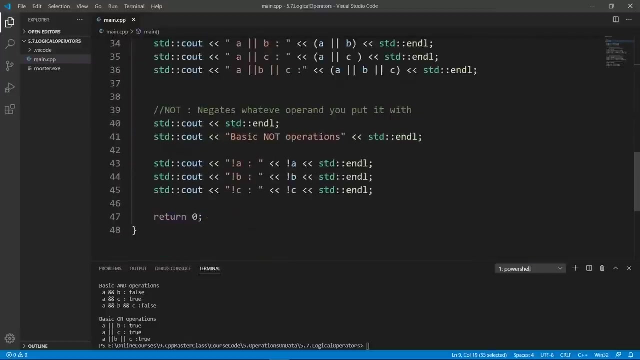 And NOT A is going to be false because A is true. NOT B is going to be true because B is false, And NOT C is going to be false because C is true, as we can see here. So let's run the application and see if 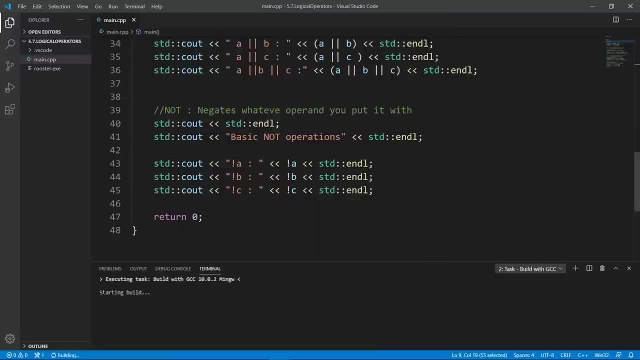 this is what we expect. We're going to run and build with GCC and we're going to run rooster and we're going to see that NOT A is false, NOT B is true and NOT C is false, And this is what we expect. 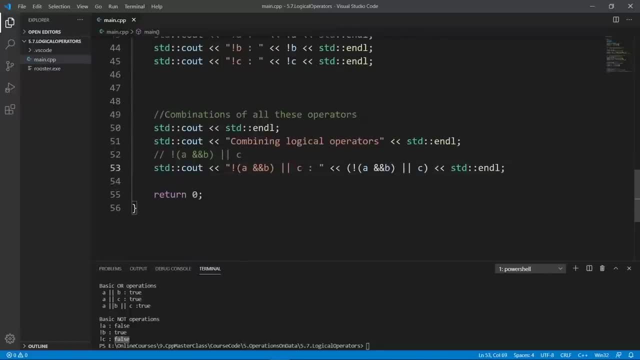 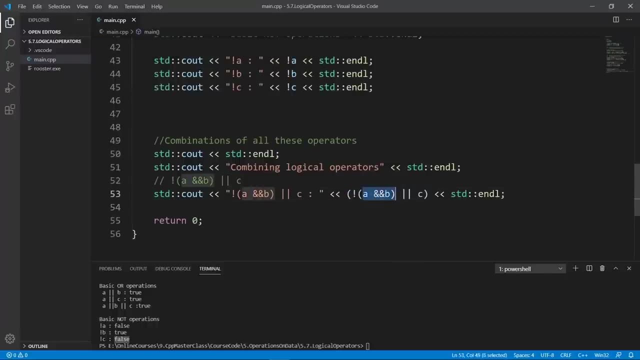 We have also seen that we can do combinations of these operators. So, for example, we can look at the expression we have here. We're going to take A and B. This is going to evaluate To false because B is false. We're going to negate this and we're going to get a true. 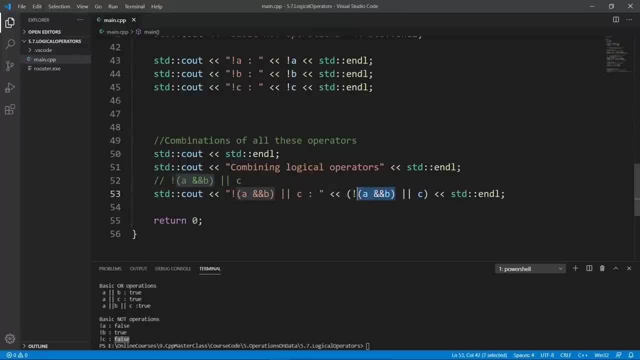 And we're going to order that with C. But because it's true, we know that the result of ordering this with anything is going to be true, so we expect this expression here to evaluate to true. If we run this, we're going to see that this is going to evaluate to true. 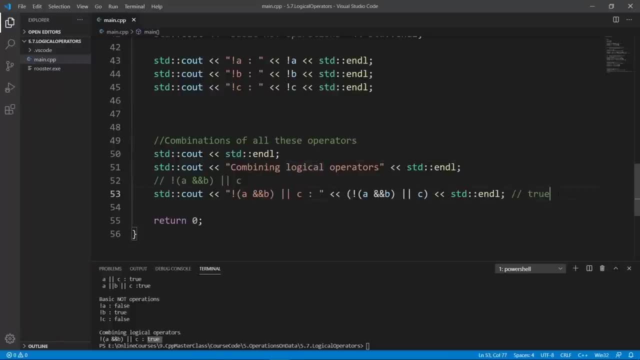 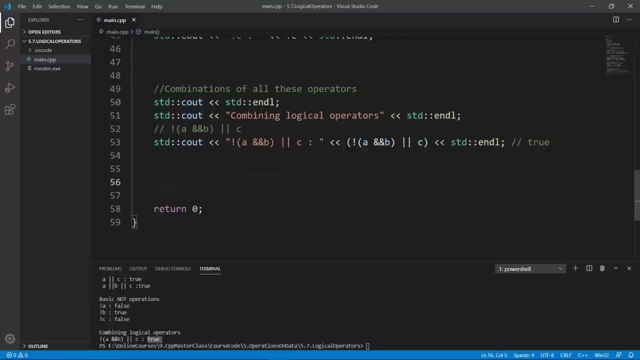 And it is what we expect. The last thing we want to see in this lecture is that we can combine these logical operators with the relational operators we have seen in the last lecture. We are going to put in a piece of code to play with this. 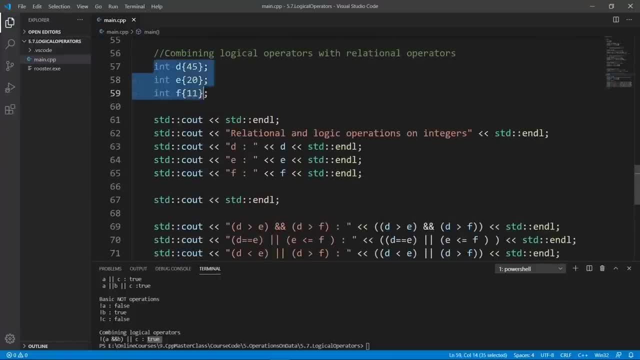 This is lengthy, but you can play with this and see what this is going to evaluate. to To start you off, we are going to do the first one together. So it does test if D is greater than E. And if you look here, 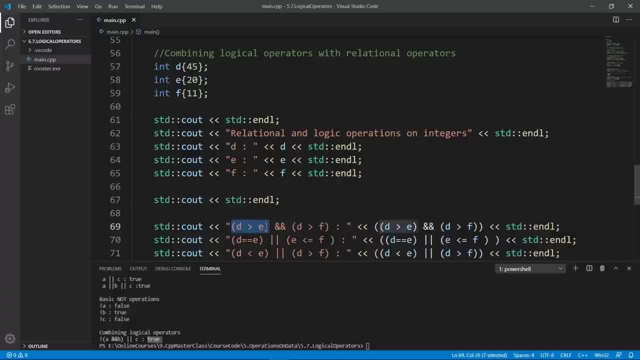 45 is greater than 2. And 20.. So this is going to evaluate to true And we're going to end that with D greater than F. The result of this is going to be true. So we're going to be ending a true and a true. 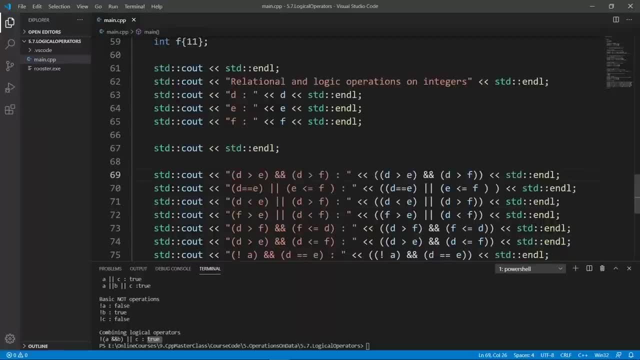 And the result of this is going to be a true And again. notice that we are wrapping this in parentheses to avoid problems with the compiler being confused with what we are trying to print. This is going to get rid of the otherwise ugly problems we might have to deal with if we didn't wrap this into parentheses like this. 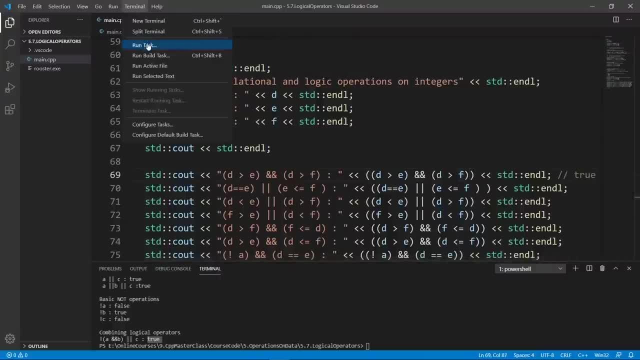 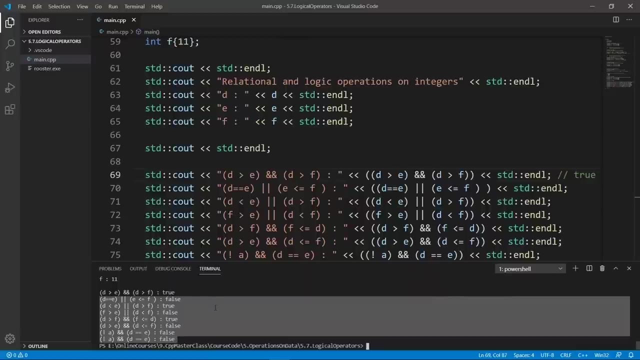 So we expect to see a true here And we're going to build and run the task to build with GCC And we're going to run rooster. And if we look at the first thing here, this is going to be true And you can try and do the other ones in your mind as an exercise. 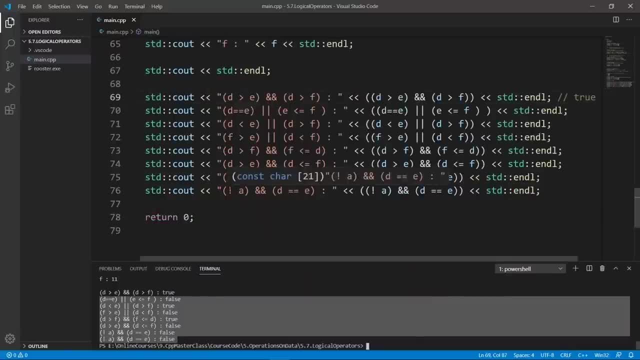 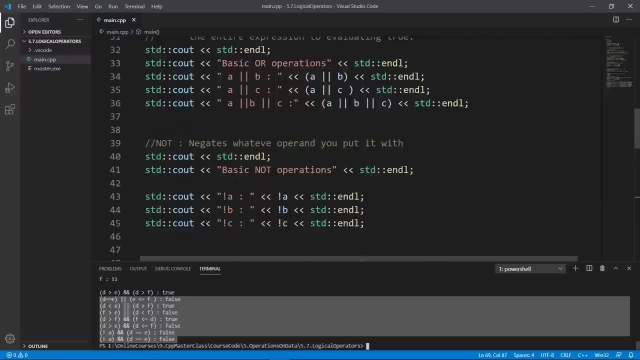 And if you have a problem, don't hesitate to ask me. I am going to do the best I can to help you out. this is really all we set out to do in this lecture. i hope you have a better understanding of these logical operators again. you don't have to really memorize them all. you have to. 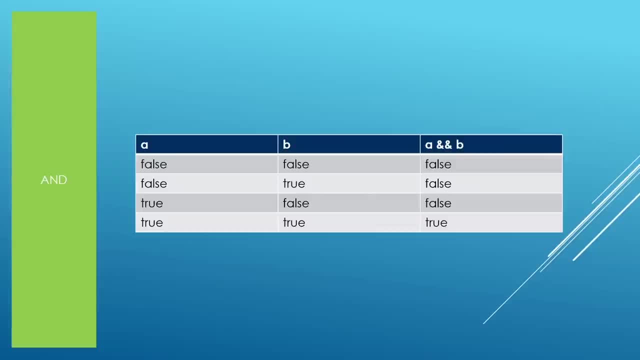 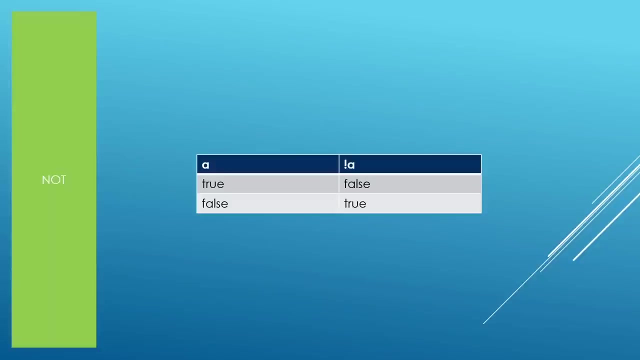 do is consult the tables and you're going to basically know the result of your two operands, depending on the values you have inside for and or and the not operator. we are going to stop here in this lecture. in the next one we're going to see how we can format our output to make it really. 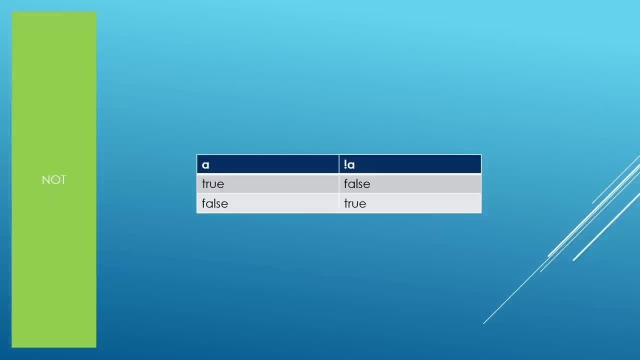 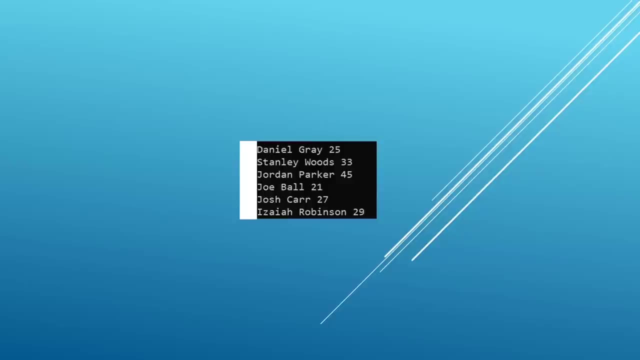 look. better, go ahead and finish up here and meet me there. in this lecture we're going to look at output formatting in c++ and this is a way we can format stuff we send to the terminal through sddc out and make them show up better. as an example, let's say we have a table here that has 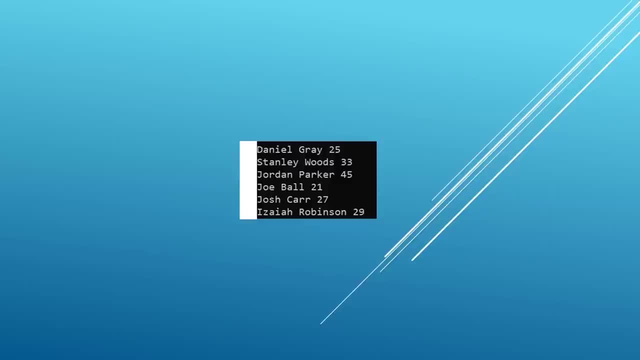 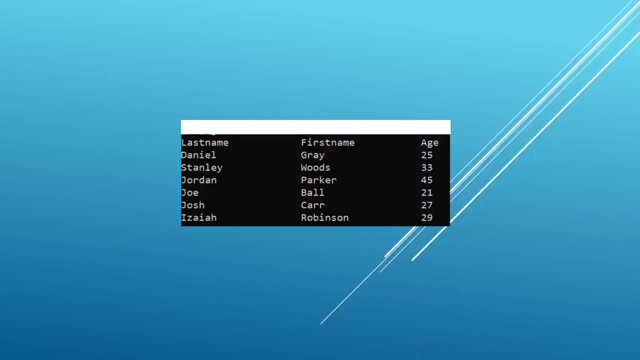 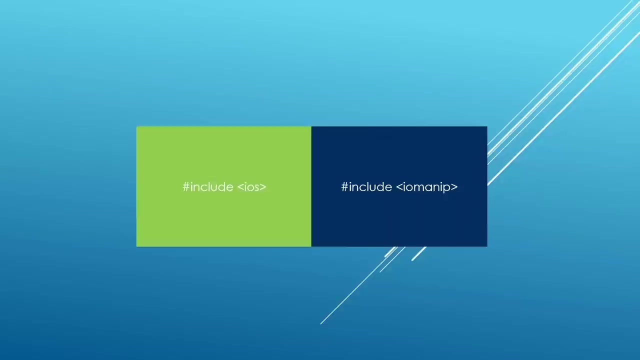 names and ages, and you see that they are are are cramped and through output formatting we can take this and turn this into this and hopefully we agree that this is better. there are a set of tools we can use in c++, and those we're going to. 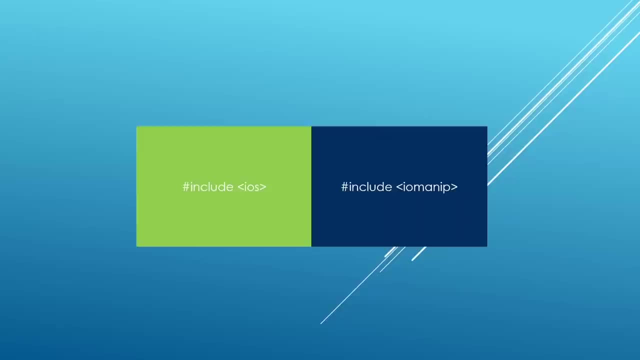 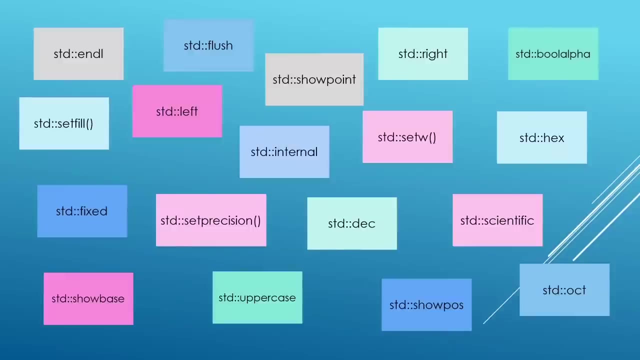 be using in this lecture are going to be coming from these two libraries, ios and iomanip, and there are a lot of things in these two libraries. here is a set of cards that show a lot of them. we are going to play with a lot of these in this lecture, so you don't have to worry. 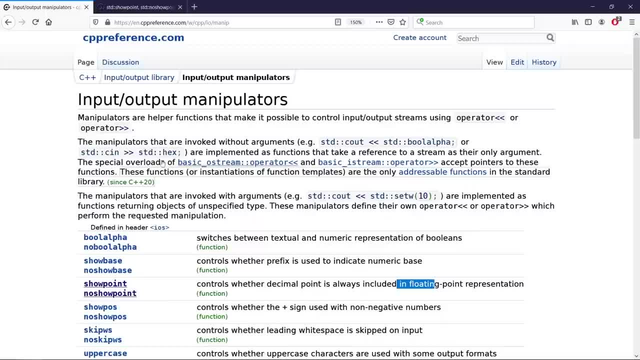 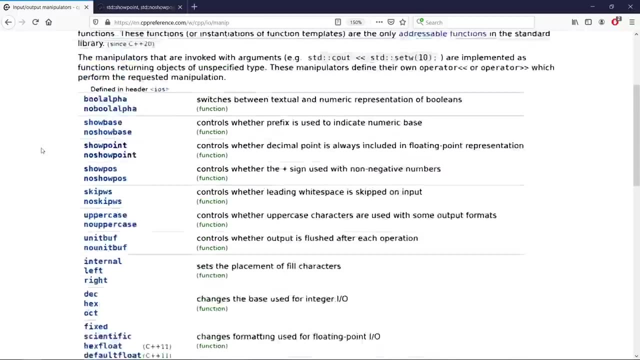 if some of them seem scary right now, before we start looking at them, i want to bring to your attention that there is a piece of documentation on these things. the link is here. the website is called cppreferencecom and you can open this up and look at some of the things we're going to talk. 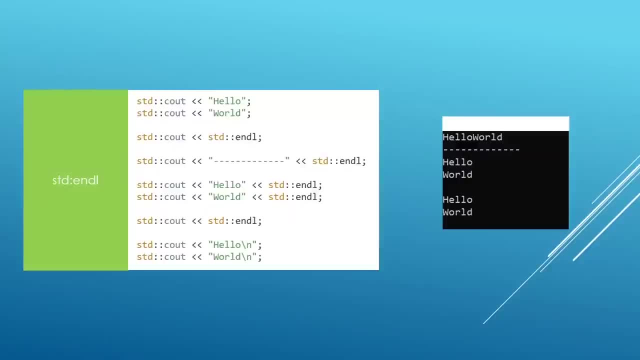 about in this lecture. okay, the first one we're going to look at is stdendl. this is not new. we have been using it all along to print out a new line character so that our stdc out statements print things on different lines. and if we don't have this manipulator, 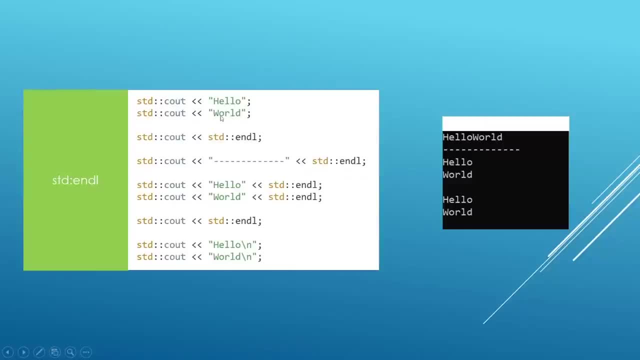 you see, here on the top we have hello and world and if we print them out they are going to show up on one line, because we are not separating the lines with stdendl down below. here we have another way. we can do this. we can push a backslash. 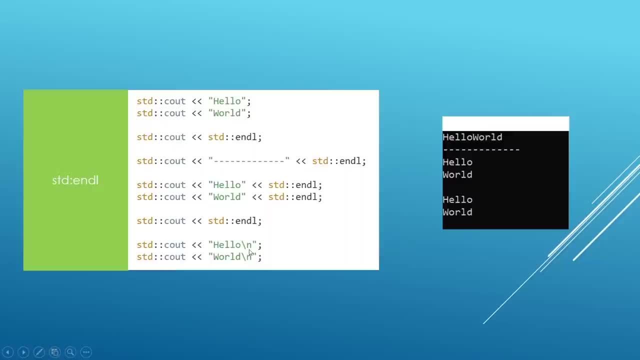 n after our text and that's going to add a new line character, just like stdendl does. okay, stdendl and slash n in here seemingly do the same thing, but they are different. but we don't have enough tools to really understand the differences right now. for now, just think of them as two things. that 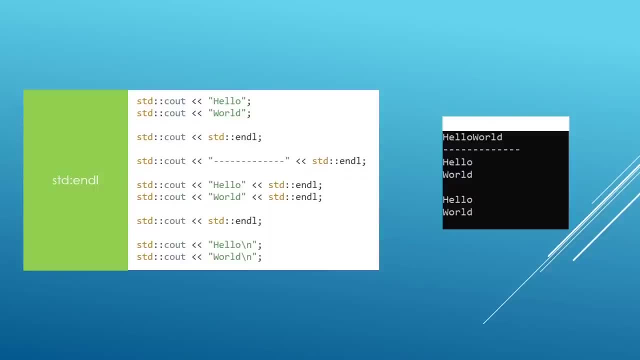 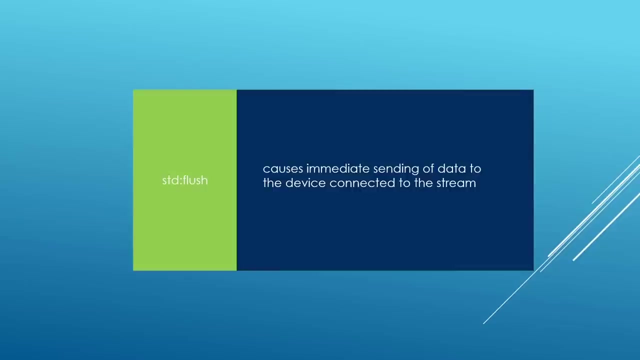 do the same thing. they print out a new character that allows your text to show up on different lines, like we have hello and world here. okay, stdendl is the first manipulator we're going to play with in this lecture. the next one we're going to look at is stdflush, and this is going to send. 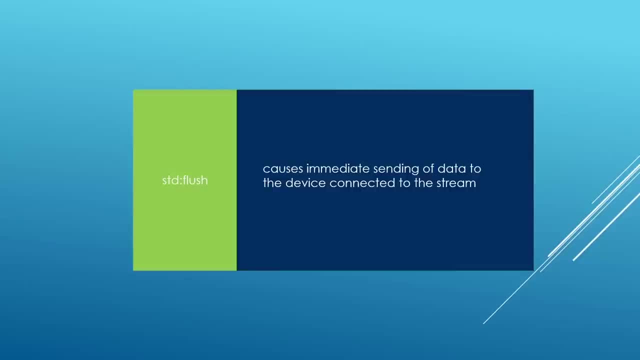 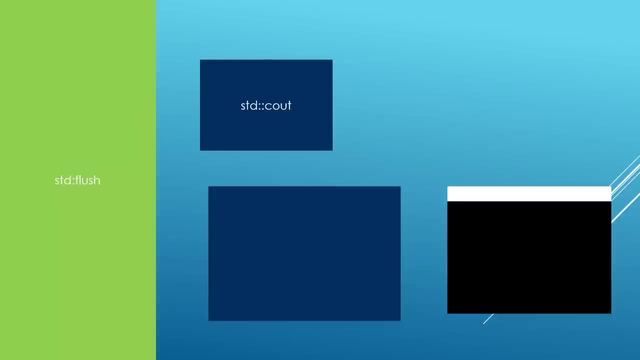 whatever is in the output buffer to the terminal. and what the heck is an output buffer? let's look at an example. suppose we have stdc out here and we want to print on this terminal and the message: how are you so? what is going to happen if the stdc out statement is executed? things are not. 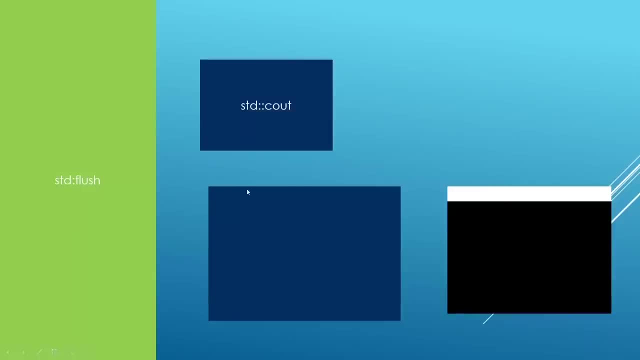 going to be directly sent to the terminal. they are going to go into an intermediary buffer. you can think of this as some kind of storage in which data goes before it goes to the terminal. and this is what's going to happen. we print out hello. hello is not going to go to the terminal. 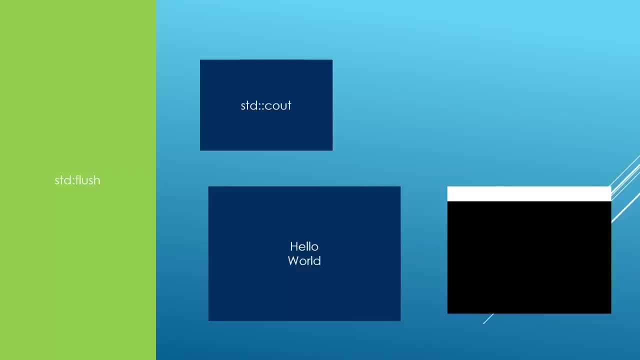 directly. we print out world. it's not going to go to the terminal. we print out the terminal and we print out. how are you? it's not going to go to the terminal, and when the buffer is full, the data is going to be sent to the terminal in one go, and this may come in handy in some situations. 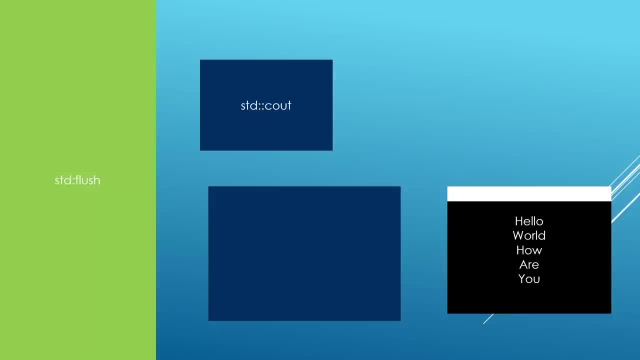 so if you want the data to go to the terminal directly, you're going to add an stdflush after your stdc out statement and we are going to play with this in a minute in visual studio code and you're going to see how this works- another manipulator we have, which is the stdc out. 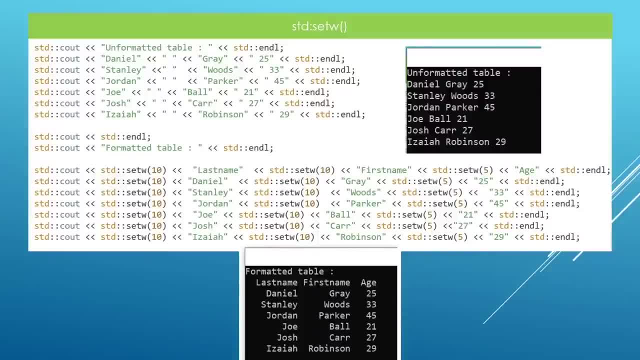 which is really cool- is set with and it is std, set w here, and what it does? it specifies a width for whatever text you want to print. here we have two examples. the first one is our table. that is not formatted well and, you see, we just print out the data and it is going to show up like we see. 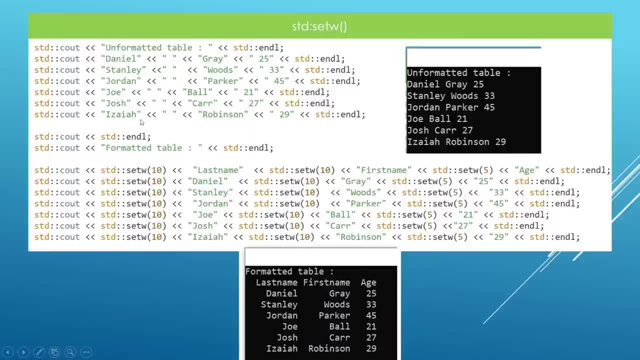 here on the right, we can use std set width to set the width of the text here and, for example, the last name here is going to show up in a field which is 10 characters wide. this is what we mean here, and we do the same for the first name and the age. and if we do this, 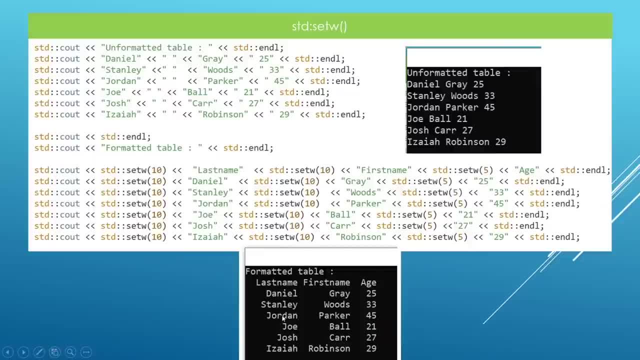 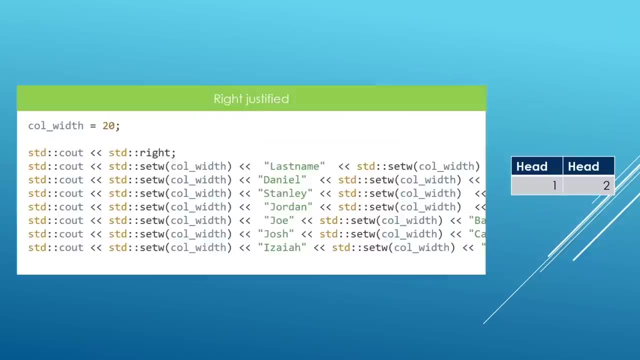 data is going to show up nicely, as we see here and again, i hope we agree that what we have down below here is much better than what we had here, which was not formatted with set width, and this is how you use this manipulator. here we can also use what we call justification to control whether our data shows up on the right. 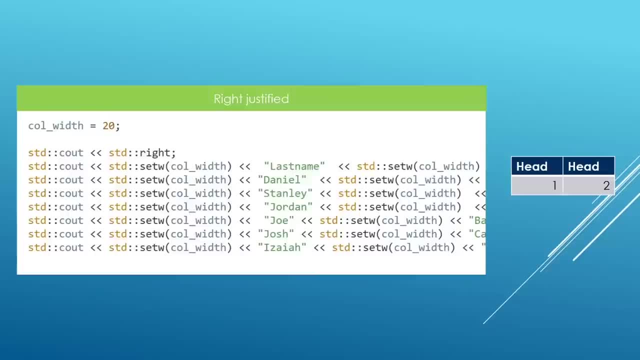 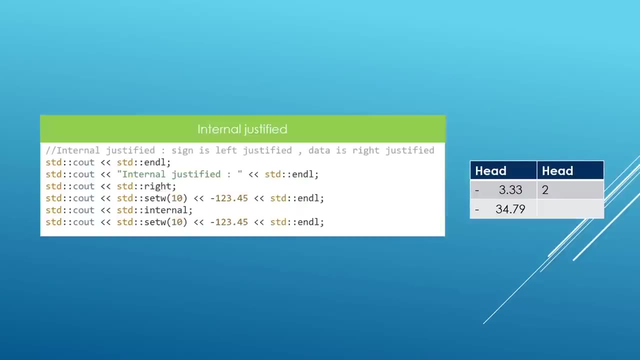 or on the left in the width that is allocated to it. for example, here the justification is std right, so the data is going to show up to the right in its respective cells. we can also use what we call internal justification, by which if we are showing a negative number, the sign is going to be left. 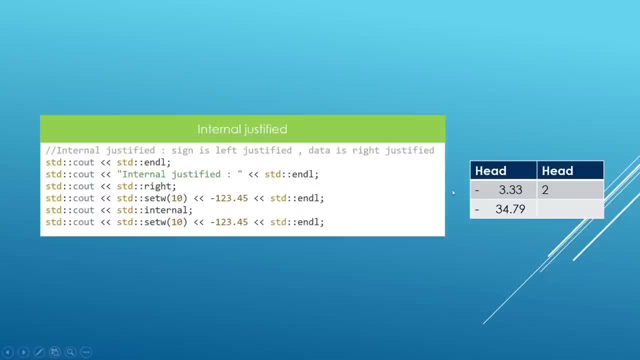 justified, so it is going to show up as a negative number and if we are showing a negative number it is going to show up on the left, but the data is going to be right, justified, and this may come in handy if you want to display some tabular data in your terminal. we can also use std set field to. 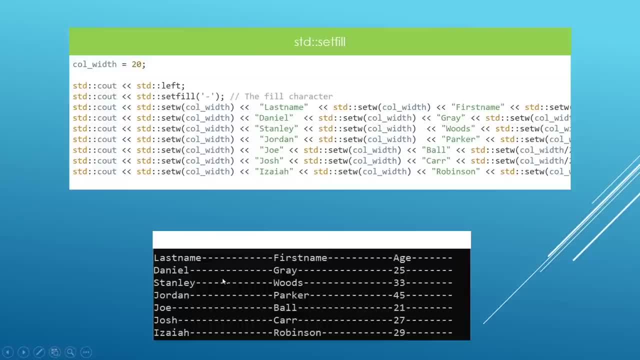 specify the field character in our empty spaces. for example, here we set the dash as our field character and the result is what you see down below. here we have seen std ball alpha, and its effect is to force std ball alpha to force std ball. alpha to force std ball. alpha to force std ball. 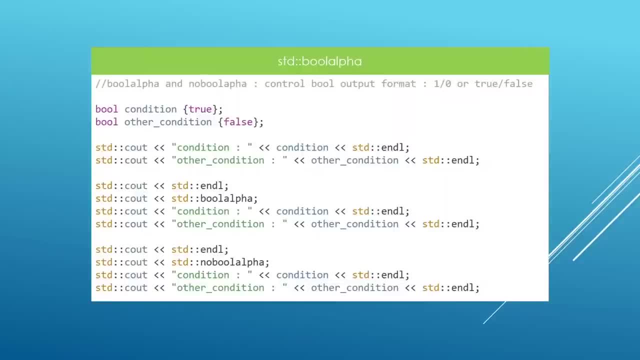 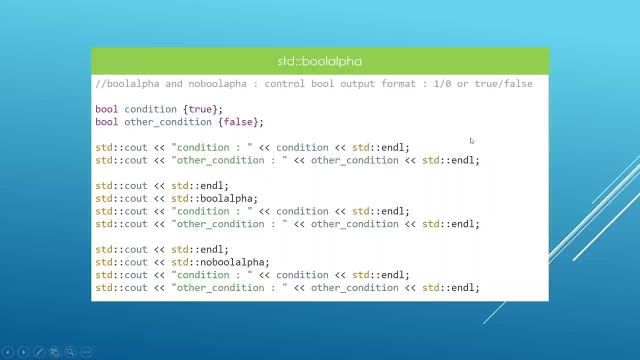 condition and data condition. if we print them out, they are going to show up as one and zero. we are going to set our manipulator here, so the data is going to show up as true and false. we can disable this manipulator here with no bull alpha and the data is going to go back to be shown in the form of 1 and 0. this is what. 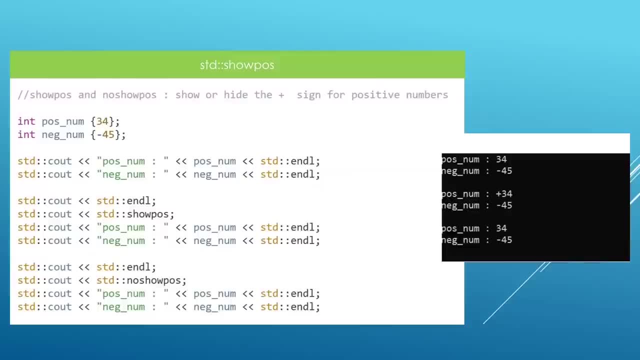 this manipulator does. we also have one to show the positive sign for positive numbers. so if we don't enable it, the data here is going to show up like this: 34 and minus 45. you see that the minus sign is going to be shown regardless of the setting you have for this manipulator. but if we 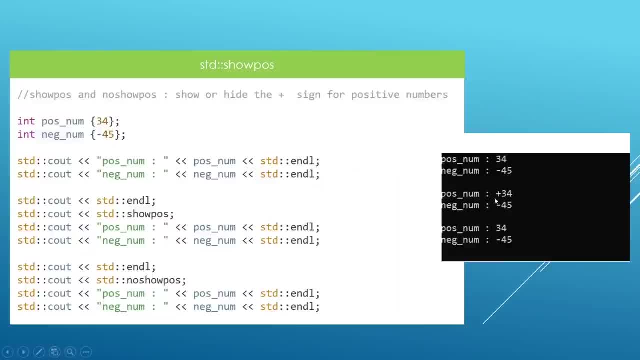 enable std- show pose, we're going to show the positive number and this may make sense for whatever application you might be doing. we can disable this with std no show pose, and after we do this, the data is going to show up in its default format that we have seen before. this is how you. 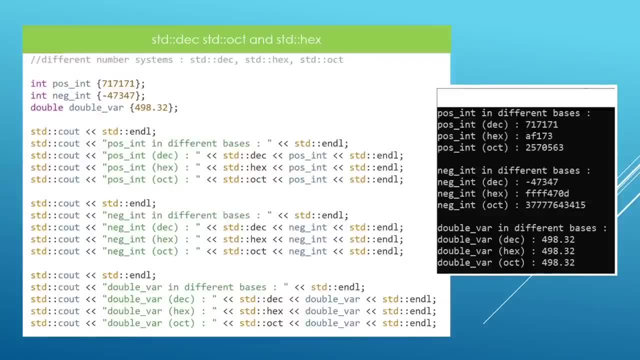 use std, show, pose. we also have manipulators to control the base in which the data is shown and we can show the data either in a decimal, in octal or in hexadecimal. if you look at the data here, we have an integer which is positive, we have an integer which is negative and we have a double variable. 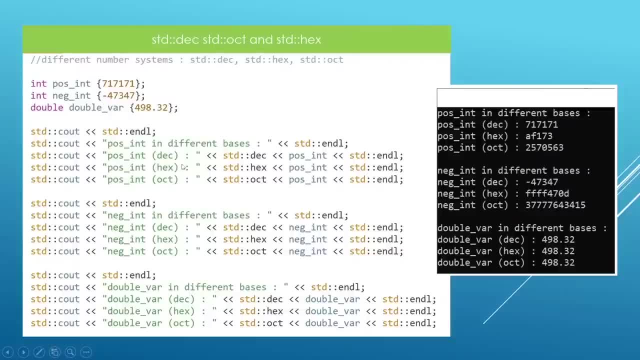 here and we have some data n for us to play with. we're going to show our positive integer in these three bases- decimal, hex and octal- and the result is what you see here, and this should be no surprise. you already know these number systems and how they. 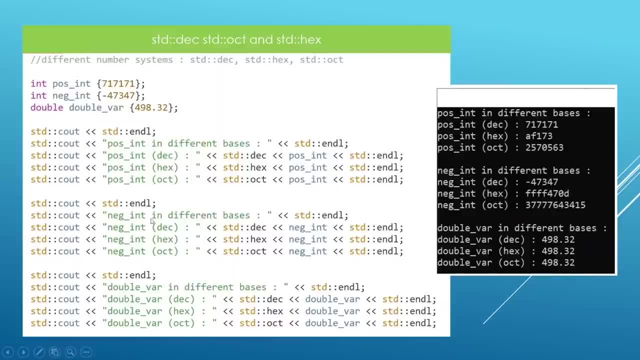 work. we can detect the negative number and also show it in different bases: decimal, hexadecimal and octal- and it is what you have on the right here in our terminal. if you go down and try to show a double or a floating point number in these bases, the result is not going to change because 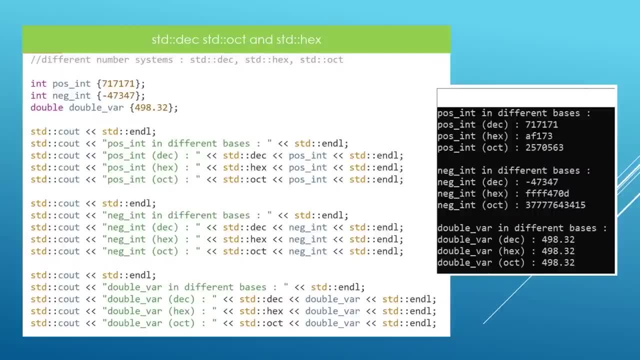 these number systems have no effect on floating point numbers. if you remember, we have seen that floating point numbers are also showing the same number, but they are not the same. in the same way are represented in memory following another protocol that is really advanced for a course like this. so we are just going to use this, but we're not going to try and understand it. 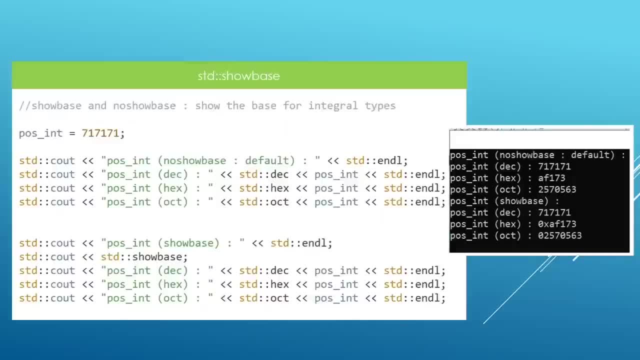 because it is out of scope for what we are doing here. we can also use std show base to show the base of our output. so here we have a positive number which is an integer, and we can show it in a decimal hex and act, and we're going to see what we see here to the right. but we can choose to. 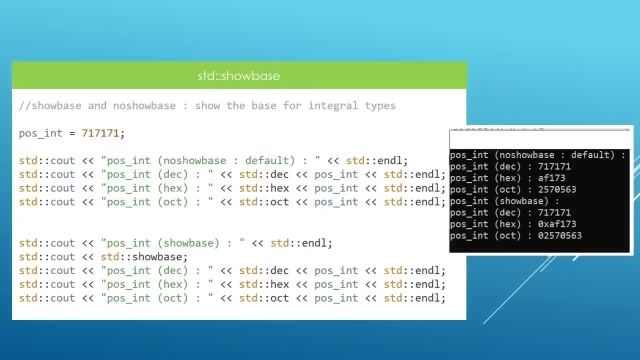 also show the base of whatever it is we output. if we want to specify that the output is in decimal, we're going to say that here. but we can also decide to show the base and we enable that with std. show base like this, and if we do this, we're going to see decimal is not going to have anything. 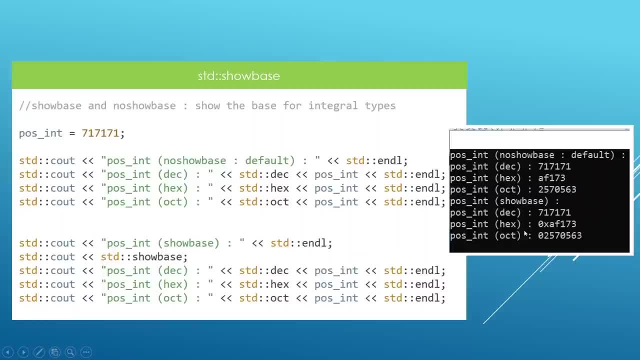 in front. hex is not going to have anything in front, so we're going to show the base and we enable that is going to have a 0x in front, oct is going to have a 0 in front and by this it is going to be. 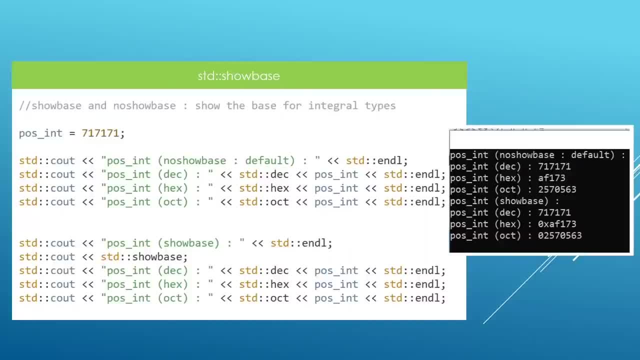 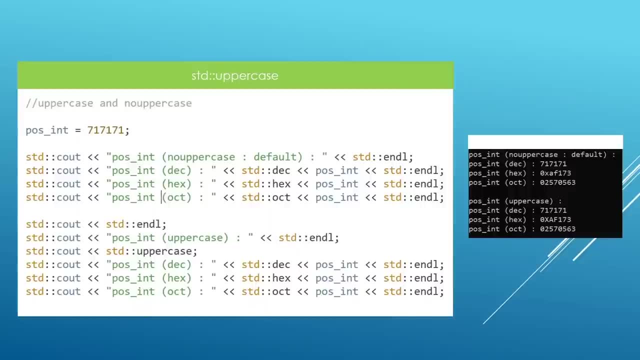 very easy to see the base in which your data is displayed. we can also use std uppercase for the data we print out to be shown in uppercase where it makes sense. for example, here we are trying to print numbers in hexadecimal here in the middle. so if we don't use uppercase, which is the default, 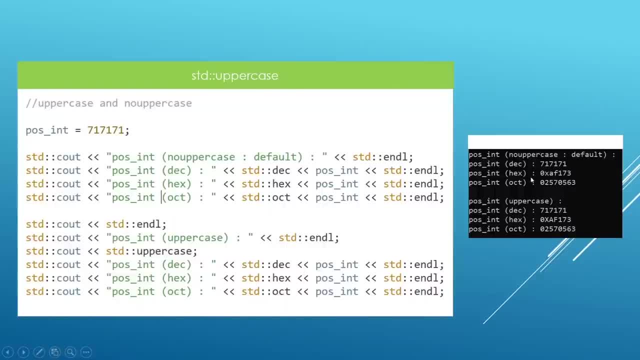 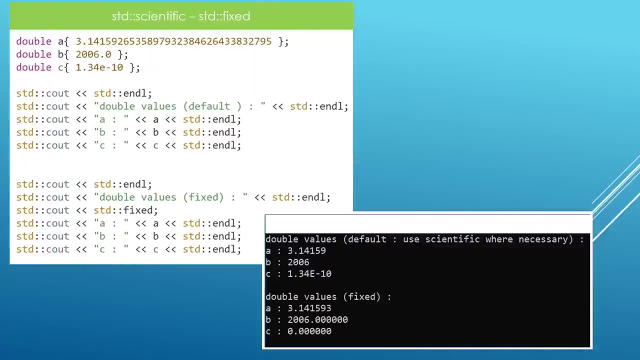 the number is going to show up like this this: you see a and f are lowercase, but if we enable uppercase, we're going to see this in uppercase, and sometimes this is going to be helpful for whatever application you are using the sun. we also have a few manipulators to control how floating point data is shown on the terminal and 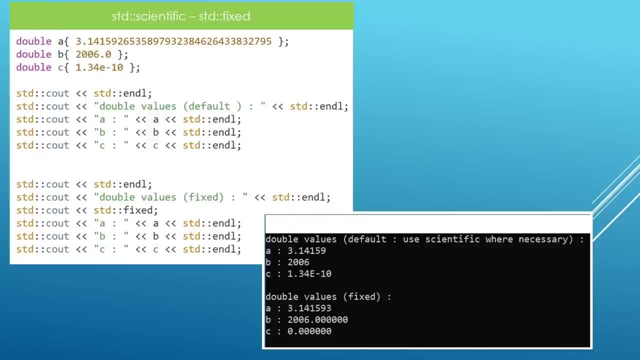 the two of these are std scientific and std fixed by default. stdc out is going to show in scientific format where necessary, and it is going to use fixed by default. so what we have here? we have three variables: a, b, c, and if we just print them out they are going to show up in this format. here, if we use fixed, we're going. 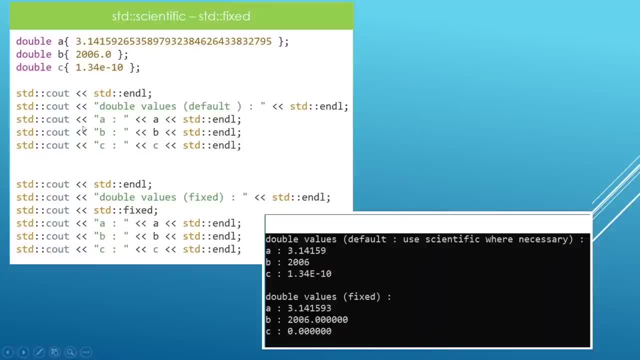 to force the output to be in fixed format and you're going to see that the third number in c here is going to show up as 0.0 and a few zeros after that, because in the precision that we have now we can't really show a number. 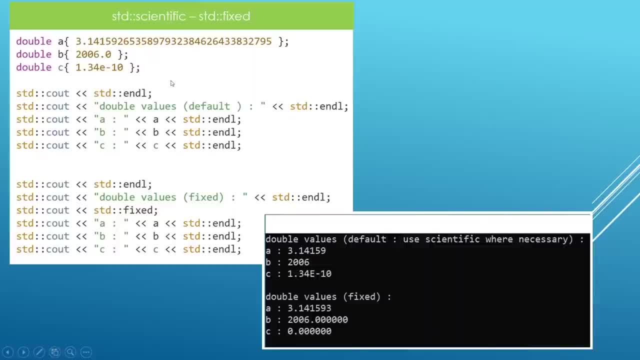 that is as low as we have here in c. again, we have seen this scientific format. this is basically 1.34 multiplied by 10, to the power of minus 10, and this is a really, really low number. so we're going to do 0.000 up to 10, and that's when this decimal point is going to show. so it's. 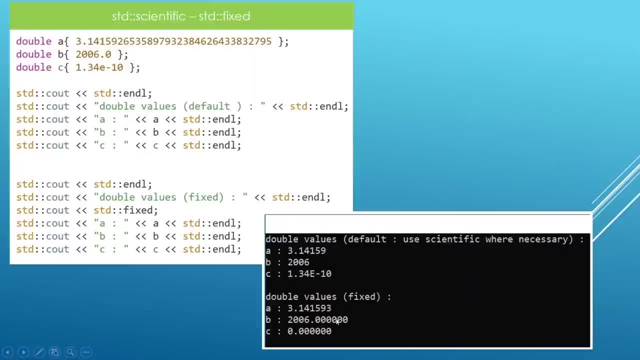 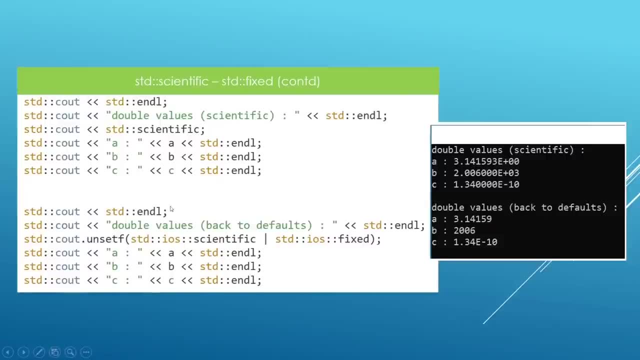 a number that is really close to zero. that's why we are showing it like zero dot zero here. i hope it is very large, bu. that means we're working with a different function. we have also shocked it in some cases because it represents an example- burkhard with the same tip as fb to see that number is 0. when we use that sort of 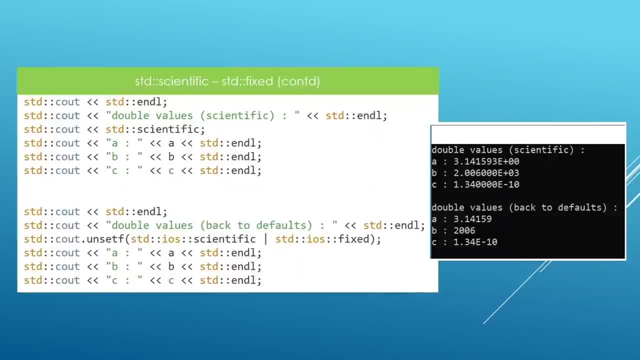 everything as output. it's itself is in the same table as fb and the data are linked now to that. scr�ar is going to be a MAT skateboard in any whatever tool theenses we will use to build that out of scope for this course. but just use this to set the floating point output format to the. 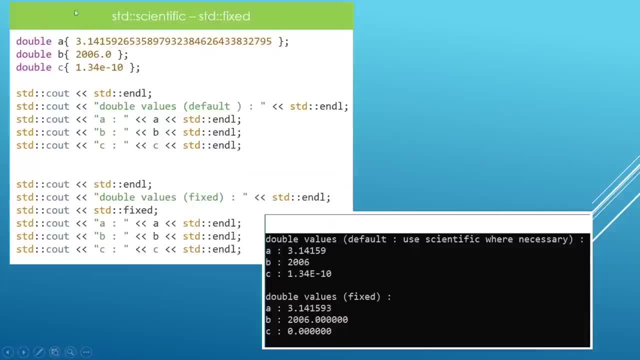 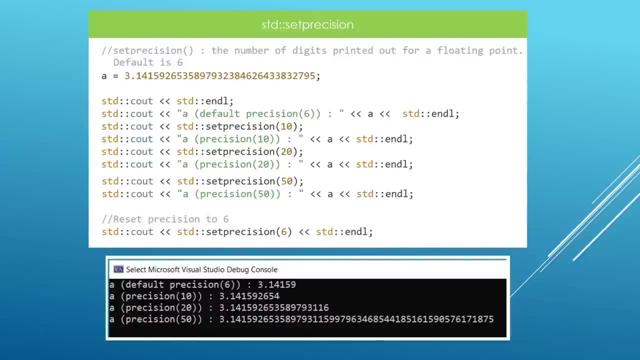 defaults, and if you do this, you're going to get whatever we had here with the defaults. you're going to see that it is the same things. the next thing we're going to look at is std set precision, which we have seen before, and this is going to set the precision with which the data is going to show. 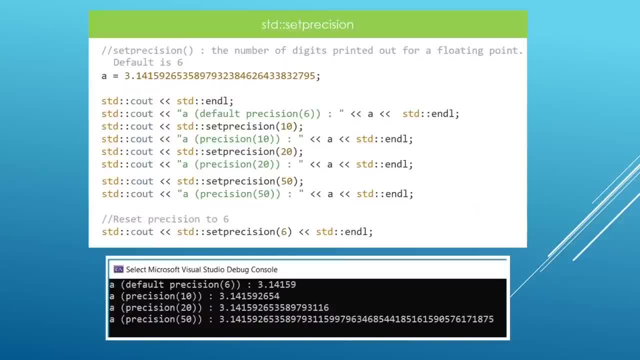 up on the terminal. if you use a precision of 10, that's what you're going to get here. here you see that we have a double number. it is a number that has a lot of numbers after the decimal point. if we show it by default, it's going to show up like this. the precision is going to be 6. 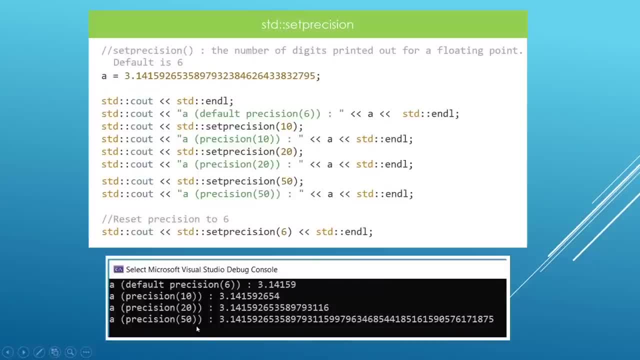 we can increase the precision to 10 to 20 and 50 and it is going to show up at whatever precision that you specify here. please know that this precision is going to be limited by the type of this a variable. if it is a floating point, the precision is going to be something like: 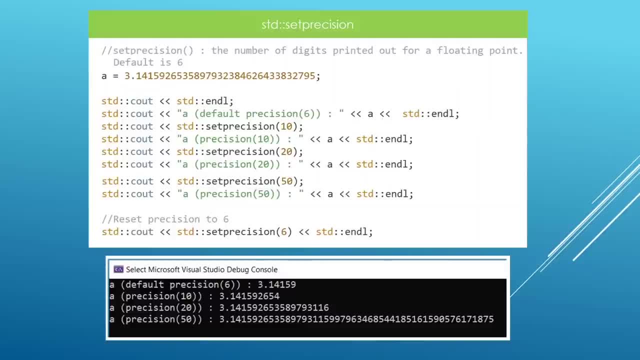 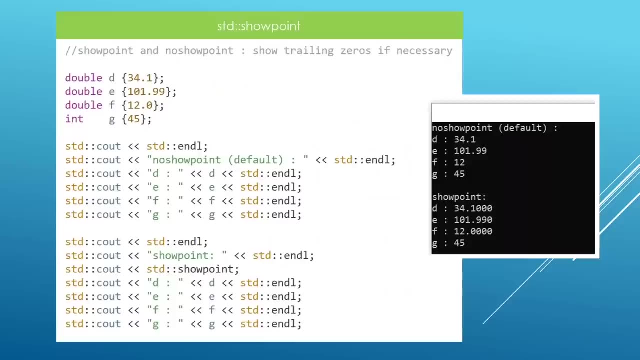 7. we have seen that if it is a double, the precision is going to basically double to something like 15, and if you have a long double, the precision is going to be something bigger than double, but it can't go below that of a double. we have seen this before. we also have 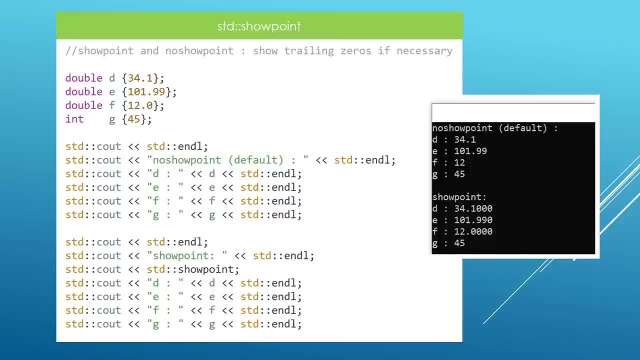 show point which is going to force showing the decimal point for floating point, but it is going to show up at whatever precision that you specify here. please know that this is going to show up as 12 in the output here, but we can use show point to force for the decimal point. 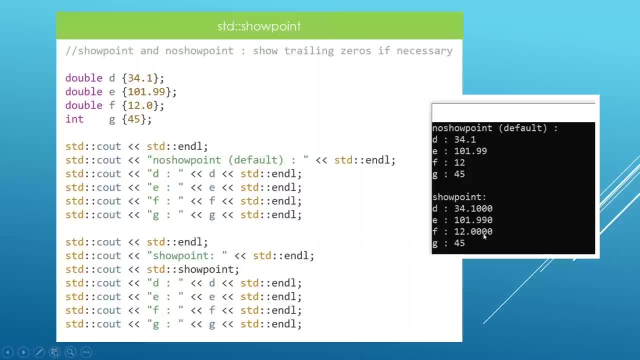 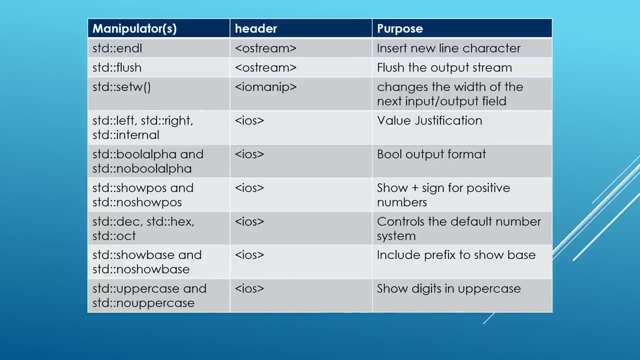 to be shown and you see that 12.00 here is shown. another side effect of this is that show point is going to force the showing of trailing zeros, and it is what we see here. in d, e and f we have seen a lot of manipulators. here is a table that is going to show where 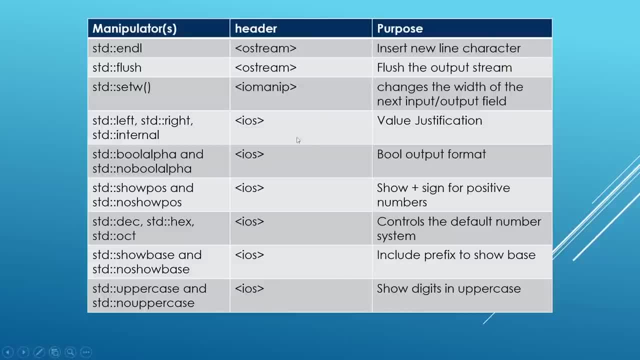 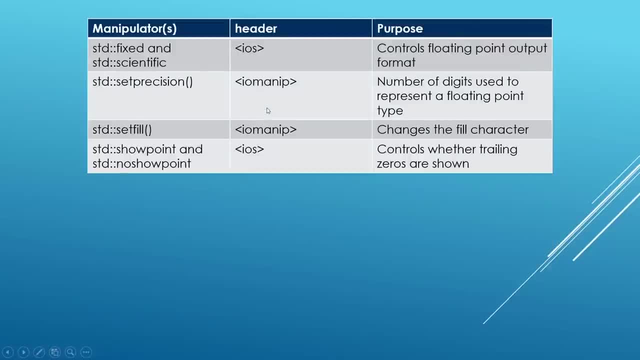 many of these are going to be living. so if you need to use set width, this is going to be living in the i o manip header and here we have a few other ones. so if you want to use a few of these things, these are the libraries that you will need to include with pound include. 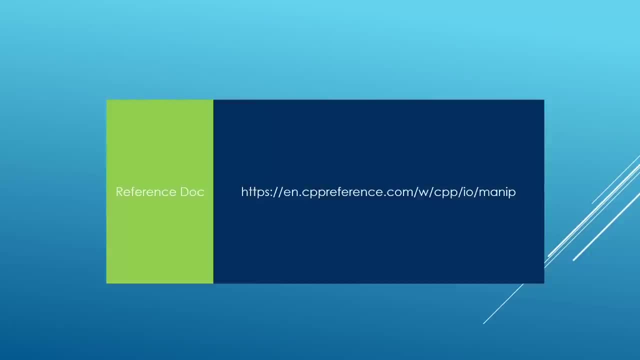 as we have been including i o stream and again the documentation is going to be the same thing, but with the front controversy. the documentation for this fence is shown at cpp reference dot com. this is the exact length and you can check this out if it helps out. 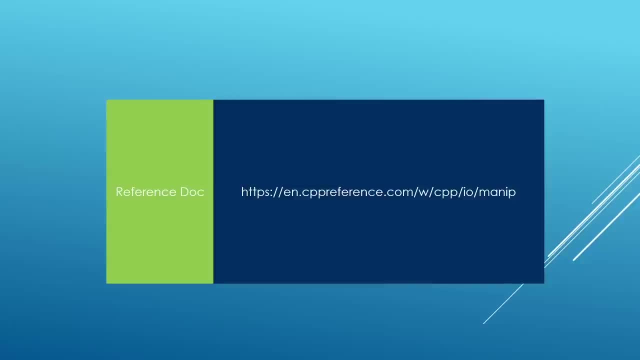 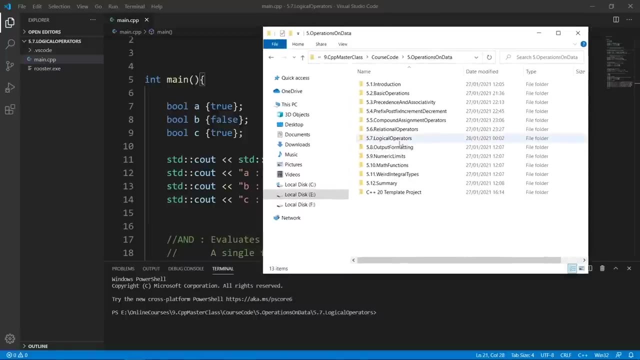 now that we have an idea about these things, we're going to go in visual studio code and actually see these in action. okay, here we are in visual studio code. the project we're going to be working on here is output formatting, so we're going to be grabbing our template. 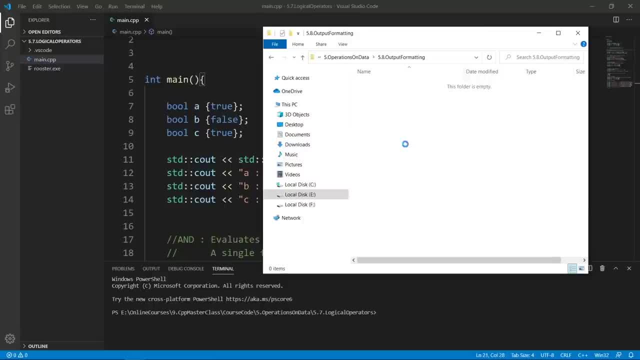 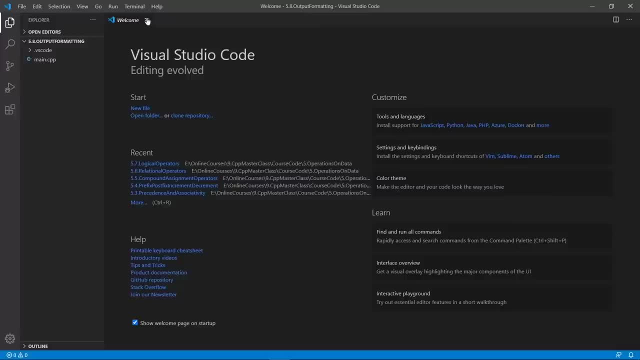 files and put those in our project code. okay, in the project code. our project code is now here and we're going to go up again and open up this folder in visual studio code. let's do that. we're going to close the welcome screen here and we're going to remove whatever it is we don't need. 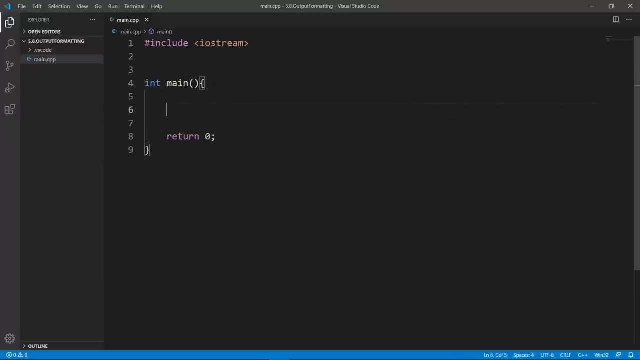 we're going to take this out and we are going to put in the first code we want to play with, and this is std endl. you don't really need a lot of explanations for this, because we've used this all along. if you don't put it out, the data is going to show up on one line and you're going to 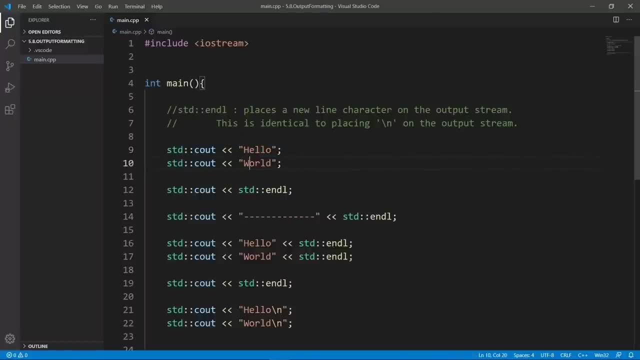 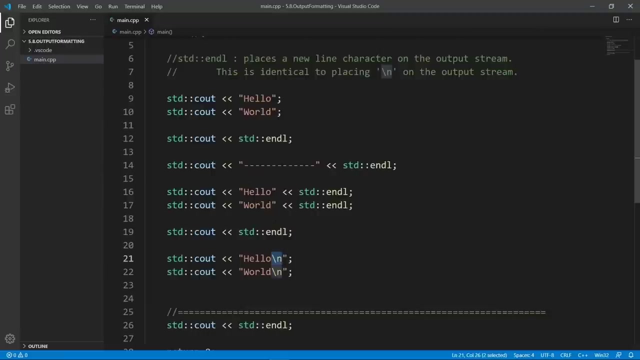 have hello, world on one line. if we put std endl like this, we're going to have the data show up on different lines. so we're going to have hello and world on different lines and it is possible to use a backslash n to achieve the same thing. but these work very differently underground and 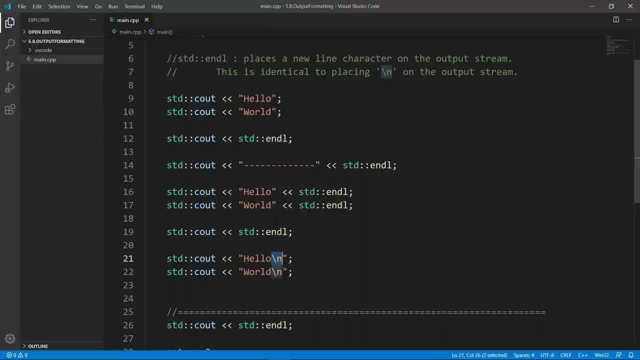 we don't have enough tools to really understand the difference, so so, so for now, just take this as the truth and know that there are differences, and the most important thing is that you recognize these things if you see them in code out there we are going to bring up. 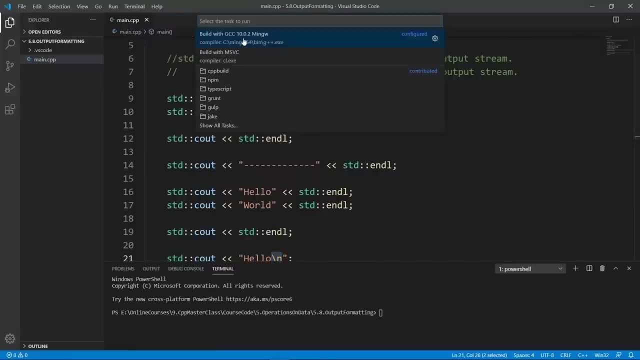 our terminal and build this with our task. that is, going to build with gcc. you're going to see that the world is going to go through and we can run our rooster binary to see the output. you see that we have hello world on one line, we have hello and world on different lines and this is a result. 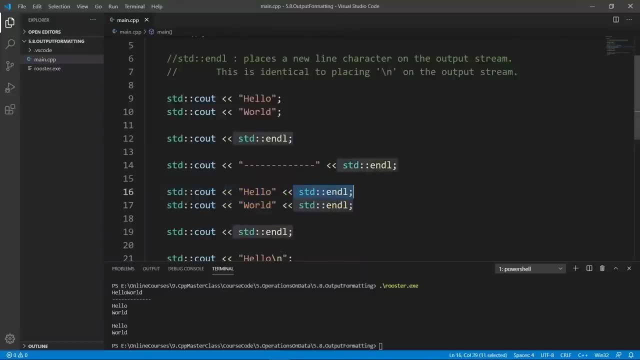 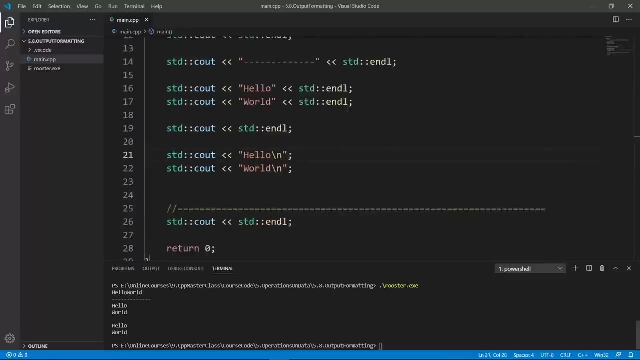 of these things we have here. you see we have std and dl. this is going to force the terminal to go to the next line and print world, and after that we're going to force the terminal to go to the next line and that's where the next text is going to show up. after that we have hello and world down. 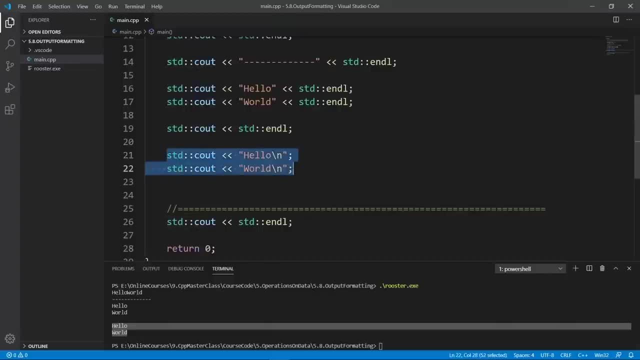 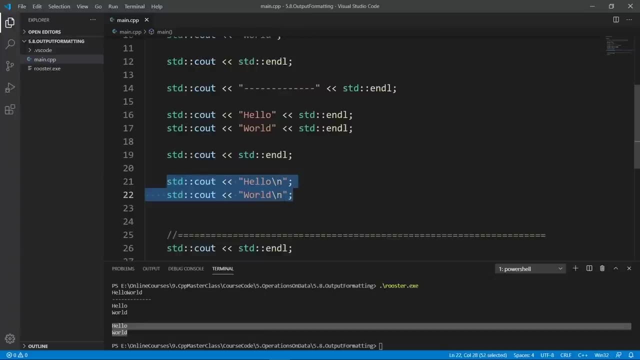 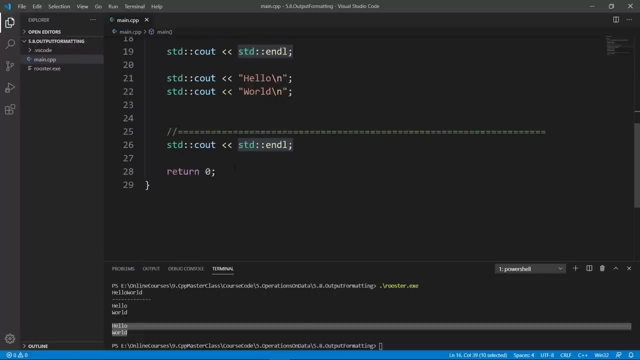 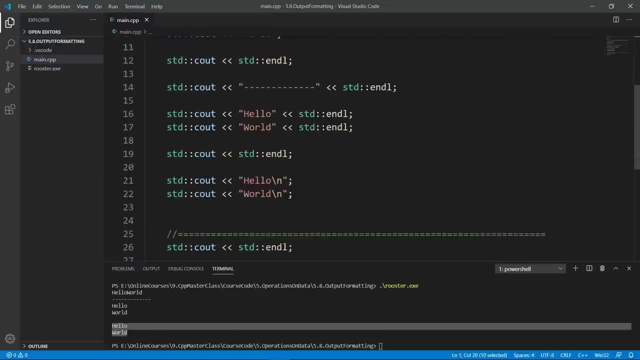 here in the terminal, and it is the output generated by the statements that we have in here, and you can see that it is going to basically do the same thing as std and dl, but again, they work very differently under the hood. okay, so this is really how std and dl works, and you get access to it by including the iostream library here. the next thing: 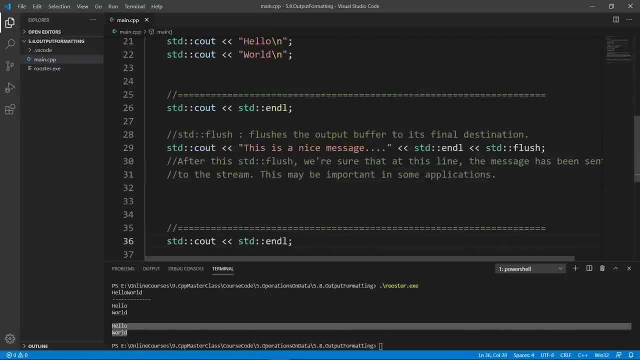 we're going to play with is std flush. this is going to flush the output buffer to its final destination and that's going to be the terminal. in this case, and if we add that to our stdcl statement like this, this is going to be directly sent to the terminal, and this may come in handy in some applications. 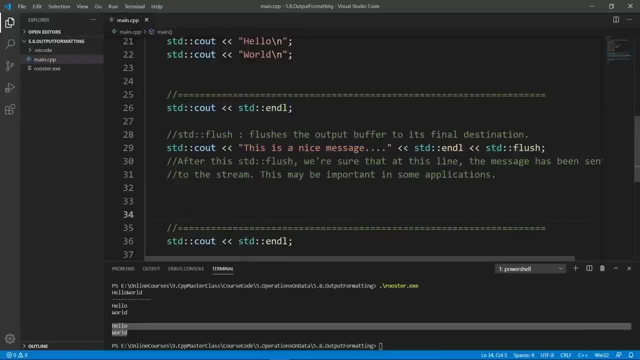 if we run this, we're not going to really see a difference, but underground, under the hood, the data is directly sent to the terminal, and we had the chance to explain this in the slides earlier. we can weld this program and we can run the program and we can see that the data is sent to the terminal. 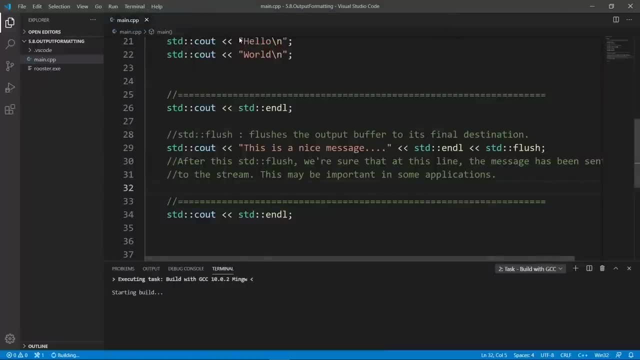 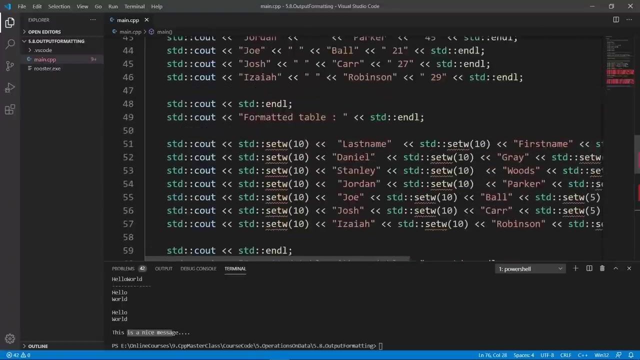 we can weld this program and i see it running. the world is going to go through. if we run rooster, we're going to see that this is a nice message is sent to the terminal. the next thing we're going to look at is set with- i am going to put in the code here because i don't want to type all this- and 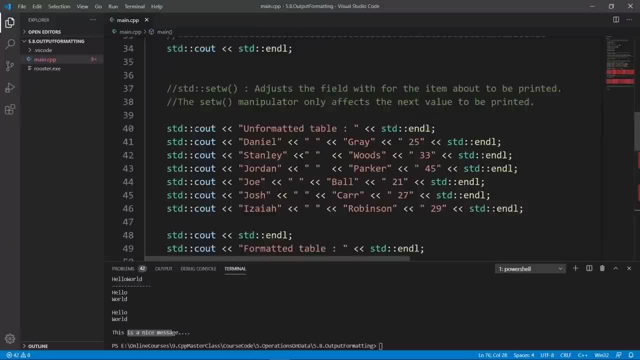 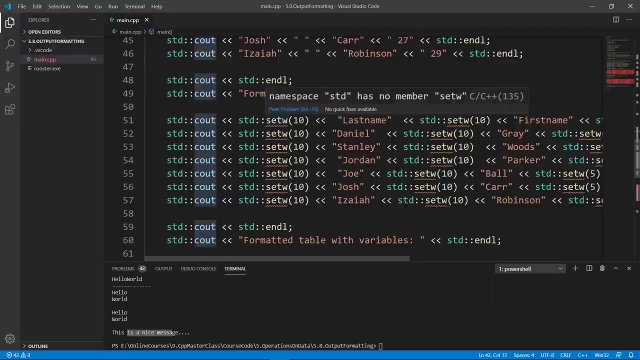 again. you can get the source code for this in the resource section of this lecture. you don't really have to type all these things. the most important thing is that you really understand how they work. okay, you see, here we are going to use set with, but we haven't really included the library. 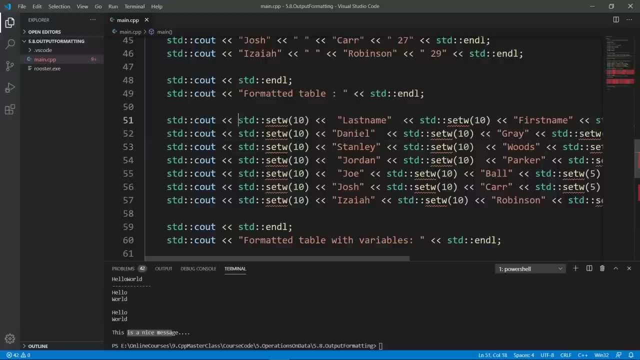 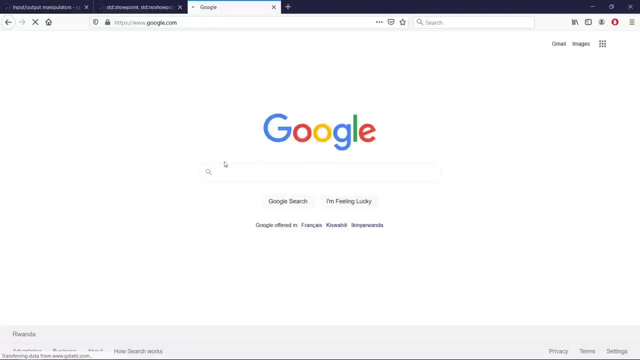 that is going to give us access to this. and if you don't know which library you will need to include to get access to this, well, you can check the documentation. and to get access to the documentation, you might want to consult your favorite search engine. i am going to go in google here and type: 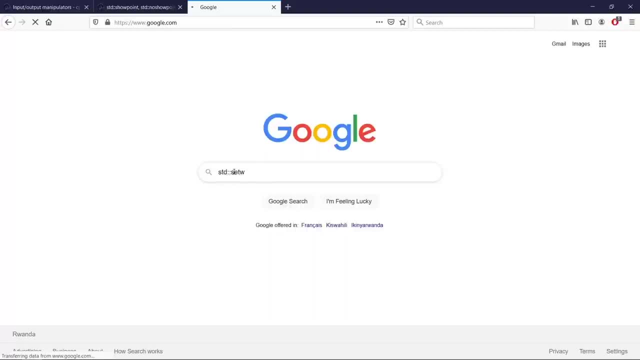 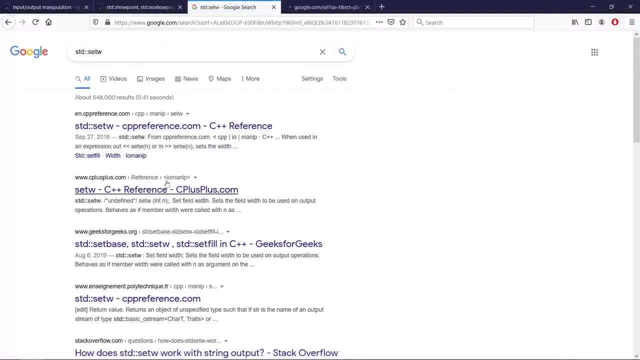 an std, set w, and i am going to search and this is going to be set with. i am going to put in the code. this is going to come up with a few entries. i am going to click on the one from cppreferencecom because this is reliable in my opinion and if we open this up, we're going to see that to work with. 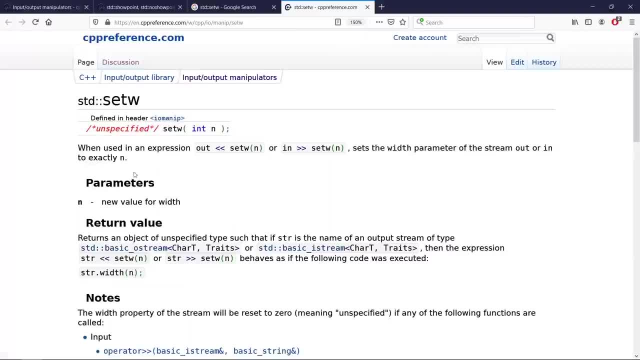 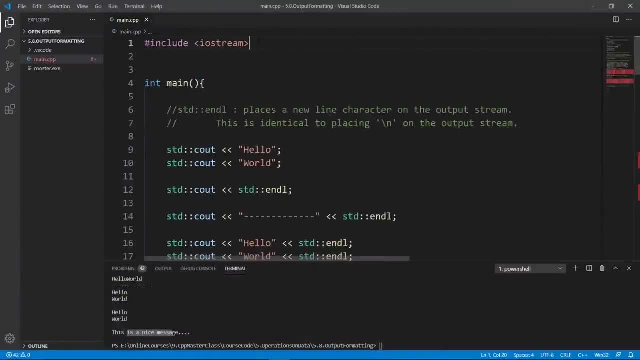 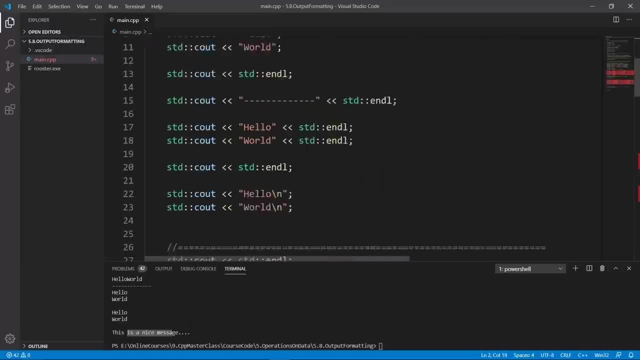 us. you need to include i o my name, so this is what we need to put in visual studio code to get rid of this problem. let's do that. i really wanted you to see this process. you can go through to know what you need to include. we're going to put this in and hopefully the arrow is going to. 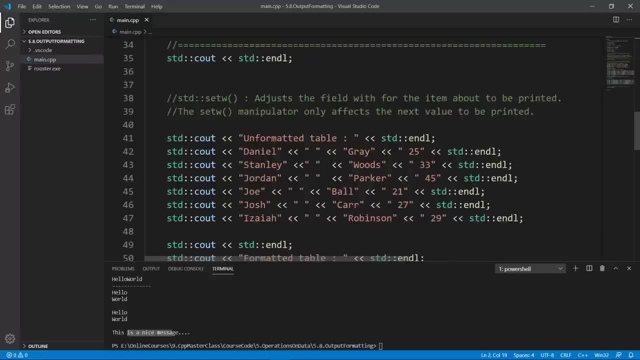 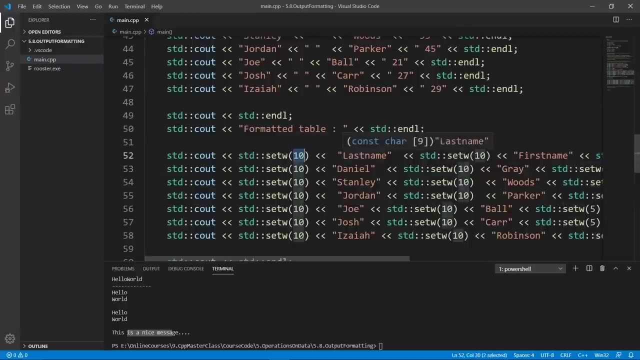 go away and we can focus on studying the effects of these things here. this is going to print and format it, so the data is going to be cropped close to each other. but we can format this using set width and if we pass in a 10 here, we are basically saying last name is going to take the. 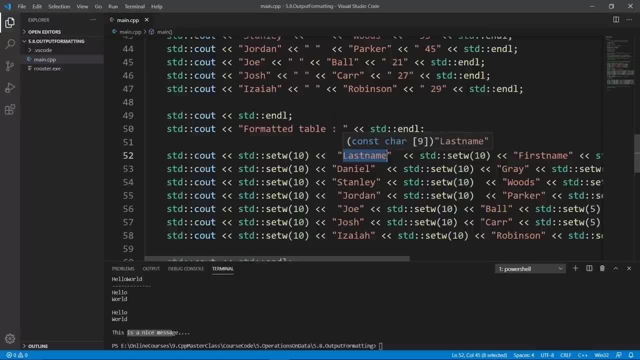 width of 10 characters, even if we don't really have 10 characters in this. so so you're going to have spaces fill the remaining spaces, so that you're going to have spaces fill the remaining spaces so that the data shows up nicely. this is really hard to say in world, so i am going to run this in a minute. 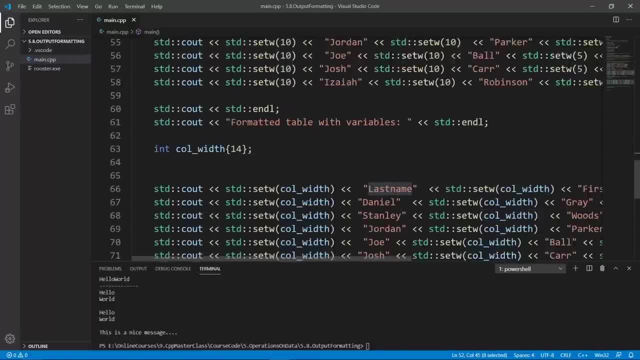 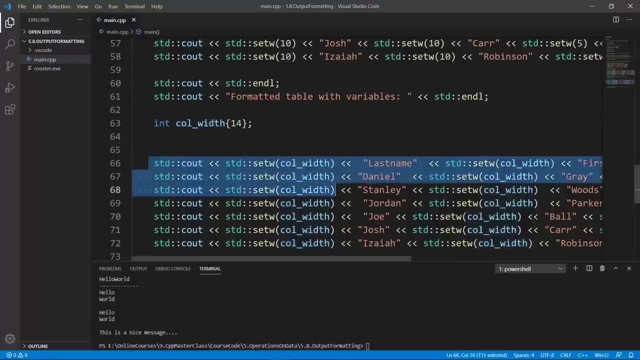 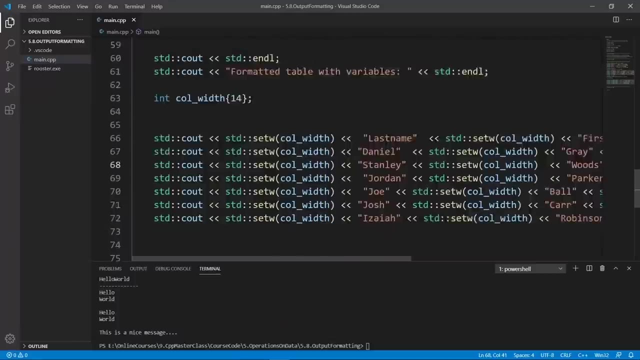 so that you can see this. but before we run, i want you to see that you can also store the width information in a variable like this, and i use that instead in your std statements. the benefit with that is that it is really easy to change this width if you happen to change your mind. 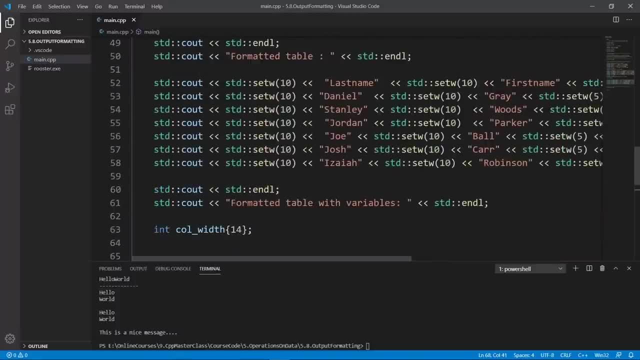 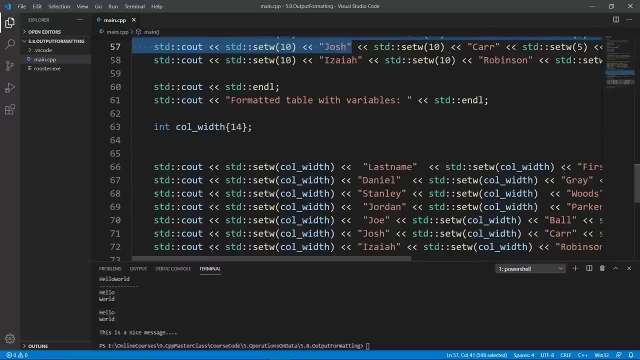 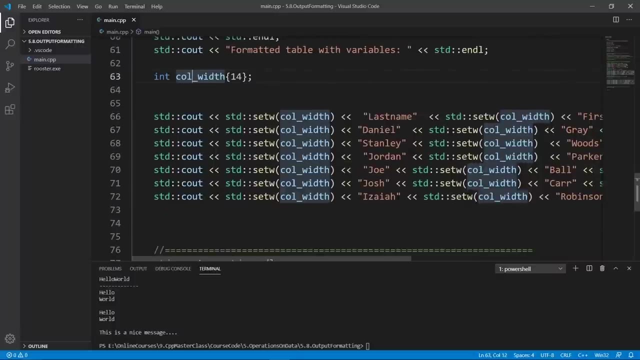 otherwise you wouldn't have to change a lot of things, and this is really bad design. i did this to show you how you can use this, but in real code you are most probably going to store your web information in a variable and that way it's going to be really easy to change and update if 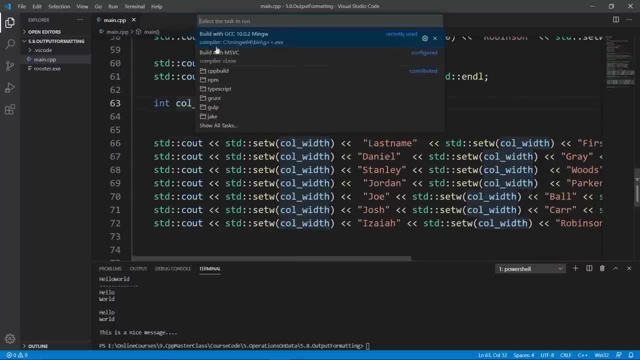 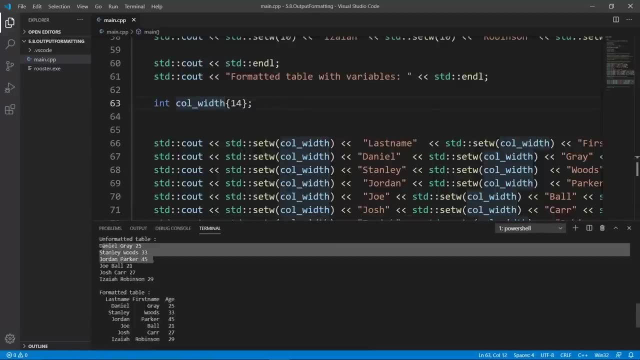 you happen to need that, we can build this program with gcc, and if we run it- let's bring this up a little bit- we're going to have our data that is unformatted, and you see that it is really ugly, but down below here we have our formatted table and it is really nice. 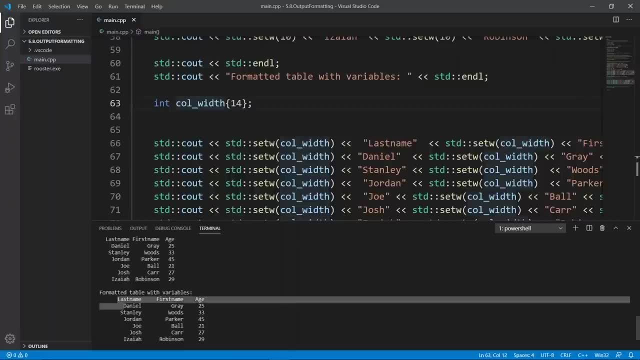 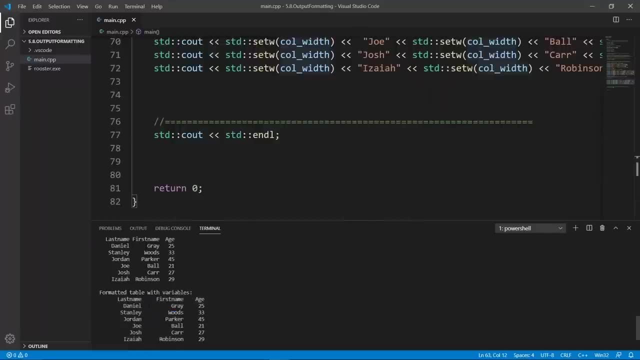 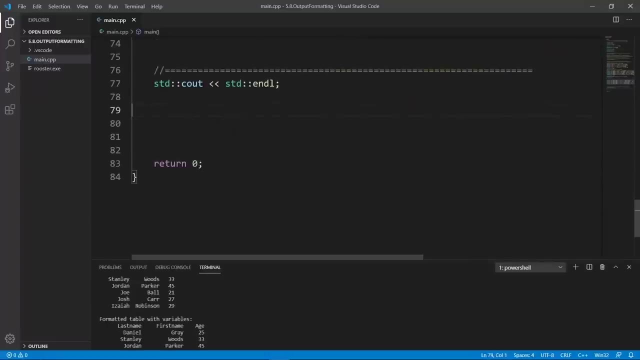 we have last name, first name and age and it is easier to see these things. we're going to see that it is possible to force the data to show on the left or to the right with justification, and we're going to look at code that does that. next, if we go down here and put in the next piece, 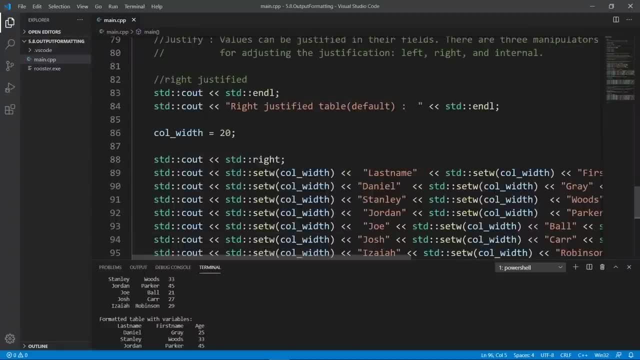 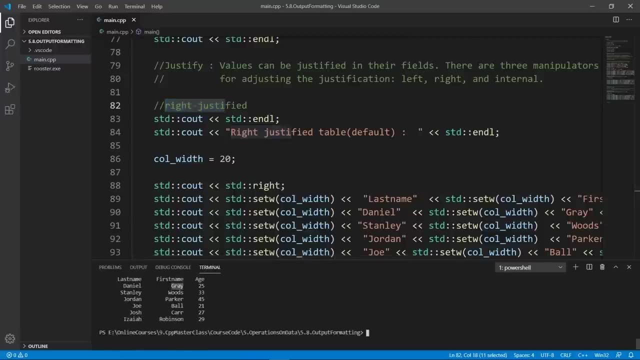 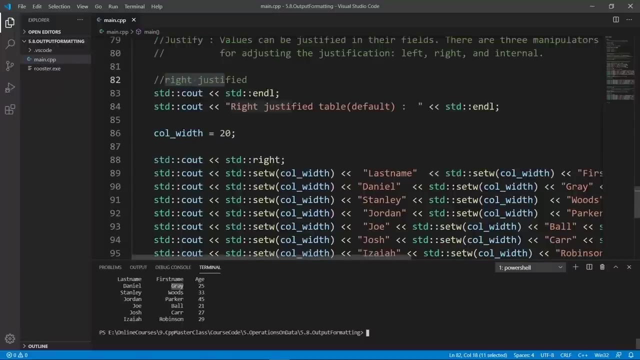 of code we want to play with. we're going to see that data is right, justified by default. but we have seen this also. you see that gray is cramped to the right of the width of the cell for the first name. so data is right, justified by default, and it is the same here if we change. 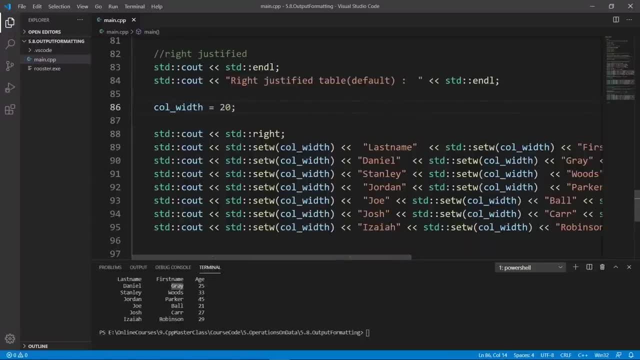 the width of our data here and try to run. we're going to have a better visualization of that. so let's run a little bit. we're going to build, the world is going to go through and if we run this, we're going to see that data is going to show up. to the right gray is, to the right woods is. 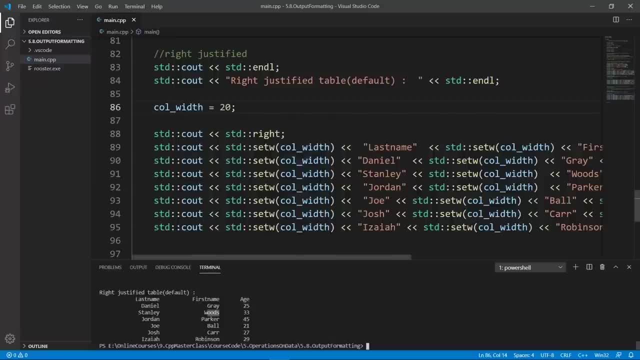 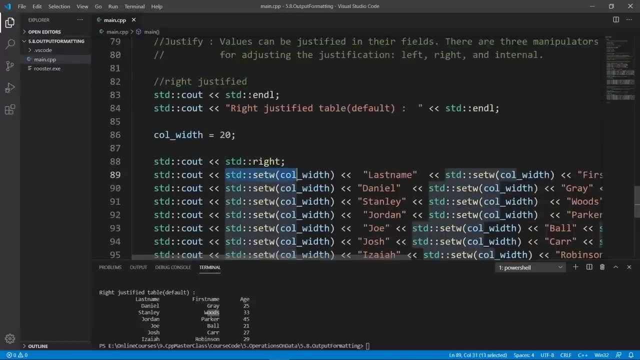 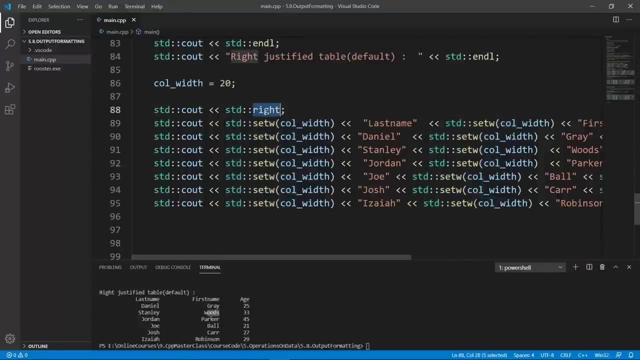 to the right, and this is the default justification. you get set width like this. you can also cause for the data to be left justified, and you do that by coming here and changing this to left. you can do that, but let's keep this in here instead for your reference, and let's put in another piece of code to justify the data. 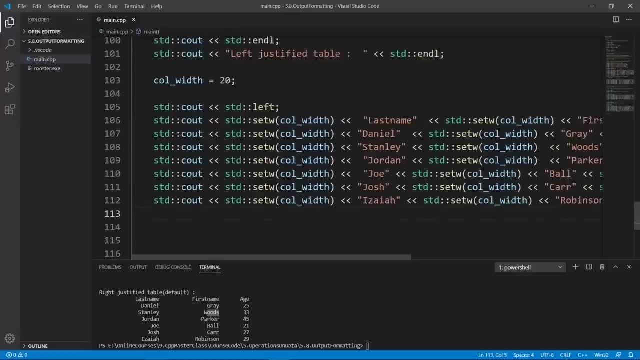 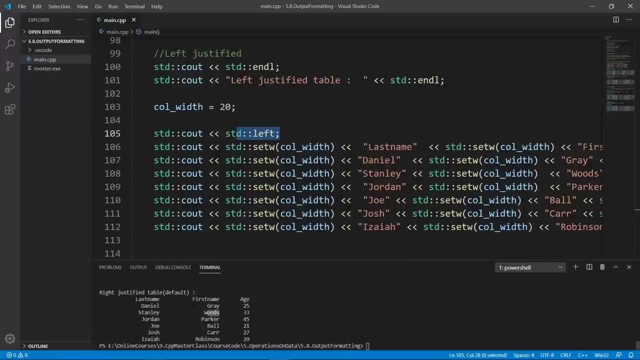 to the left. okay, let's go down and do that. we're going to justify the data to the left and if we print this out, the data here- gray- should come to the left and be aligned with the first name here. i hope this makes sense. we're going to run. 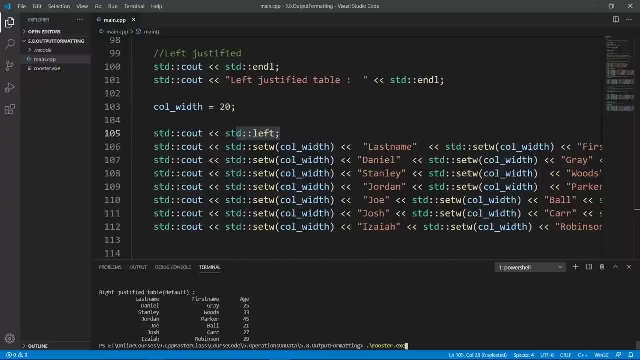 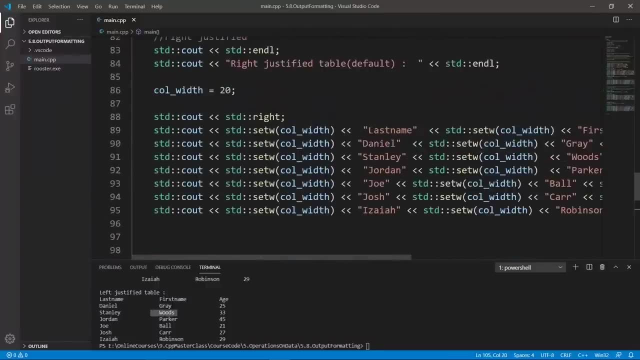 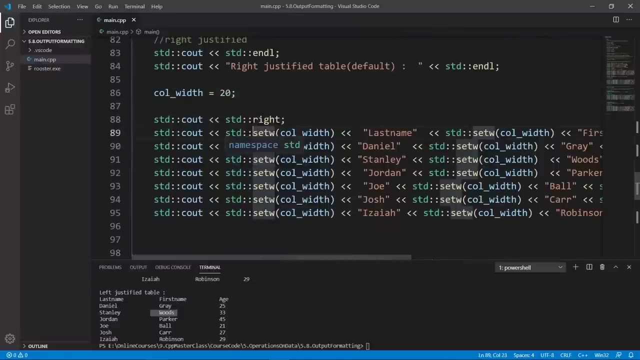 we build with gcc and if we run rooster gray is going to be justified to the left. this is the meaning of std left and std right that we just saw, and they know that data is justified to the right by default and it is important to keep the defaults in your mind. 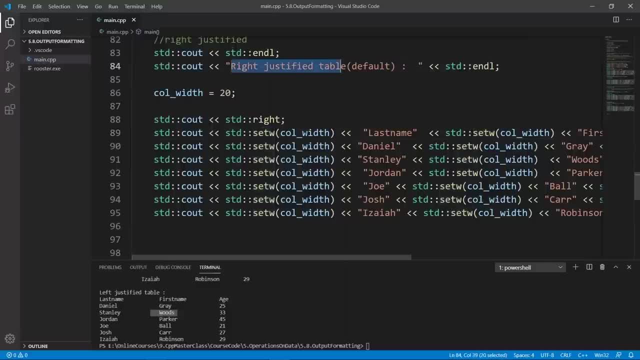 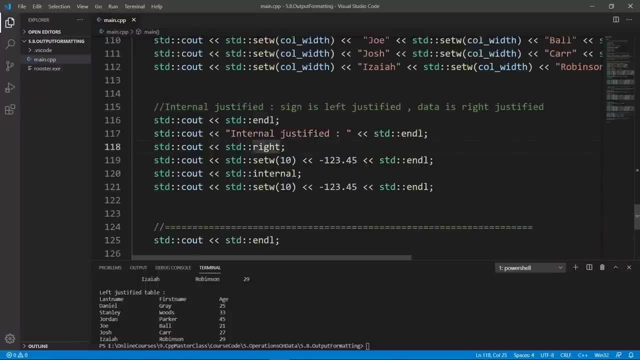 data is going to be justified to the right by default. the next thing we can do is to make our data internal justified, and what this is going to do is make the sign left justified and the data is going to be right justified, and the best way to see this is really: 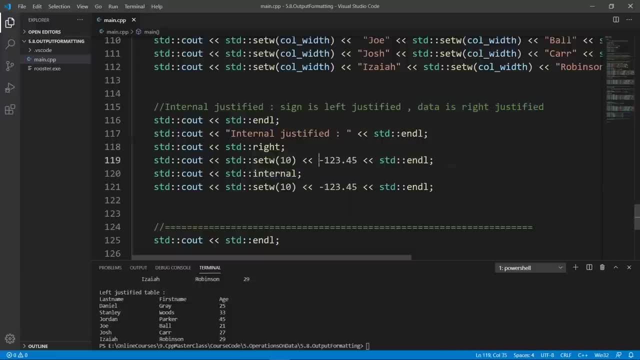 to see an example. so here we have the data. it's a negative floating point number. the width is set to 10. it's going to be right, justified, but we are also going to set the justification to internal and see the difference. let's build and run this. we're going to build with gcc and we are going to 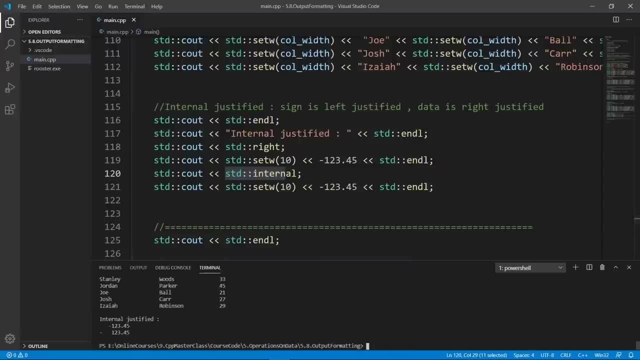 run our rooster program and if we look at the output here, you see that if we have a right justification, the sign is going to go with the data, whereas if we do internal justification, the sign is going to go to the left and the data is going to go to the right, and sometimes this is 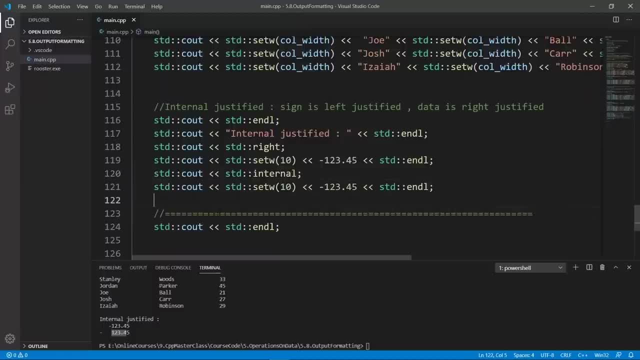 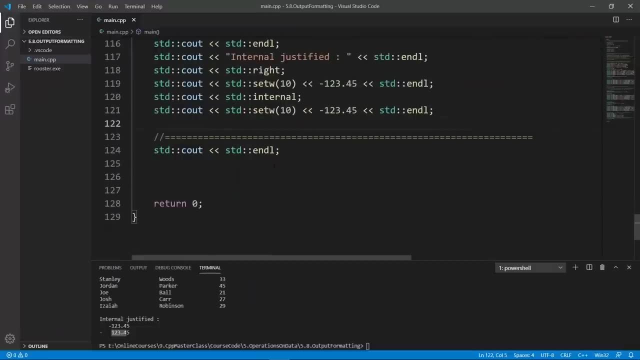 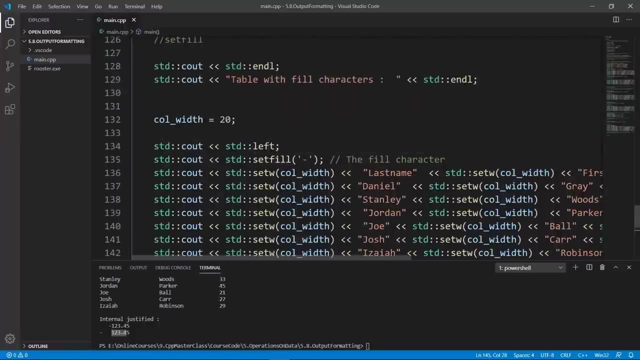 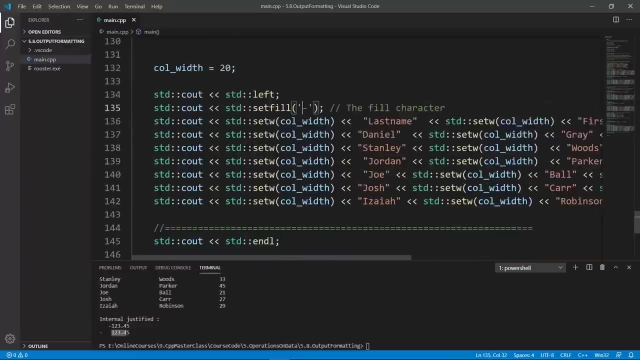 useful, depending on the application that you are using. so let's see how it works, especially in applications where you have to display tabular data on the console or the terminal. we can also specify the field character using set field, and this is really how it works. the data is going to be left justified, but we are going to fill empty spaces with a dash here and 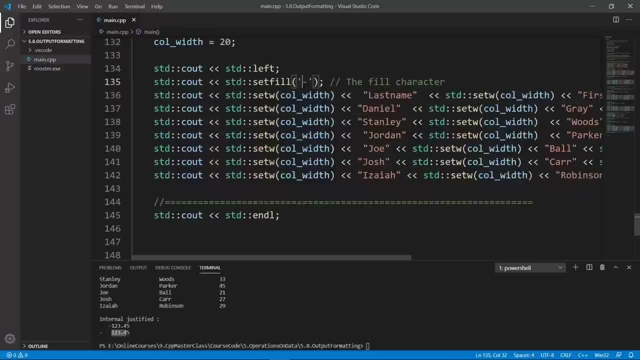 we can bring this up so that you see the entire thing, but you don't really have to type this out. you can use the code i have provided. you can use the code i have provided. you can use the code i have provided in the resources section of this lecture. you can just copy it, paste it in here and use it to play. 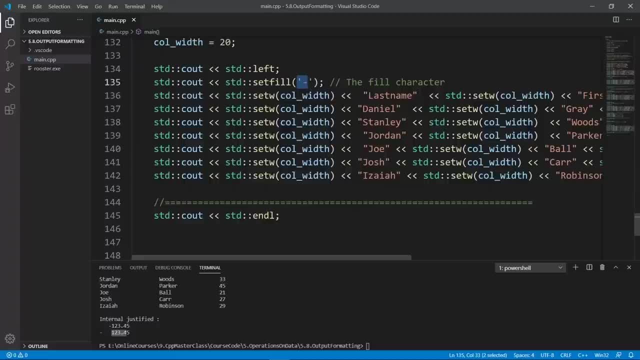 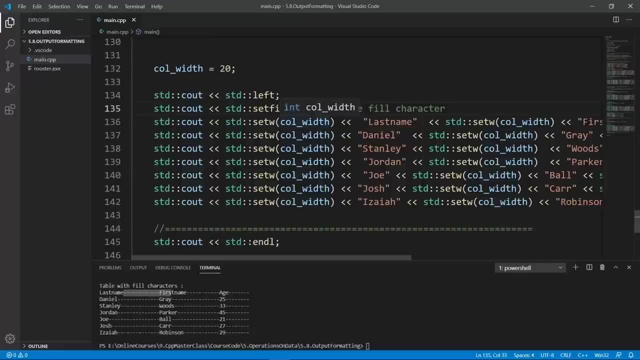 with these things. okay, with this, our empty spaces are going to be filled with this dash character. let's build and build with gcc. we are going to run this and you're going to see that we have our field character here and you can change this basically to whatever you want. if i want, i can. 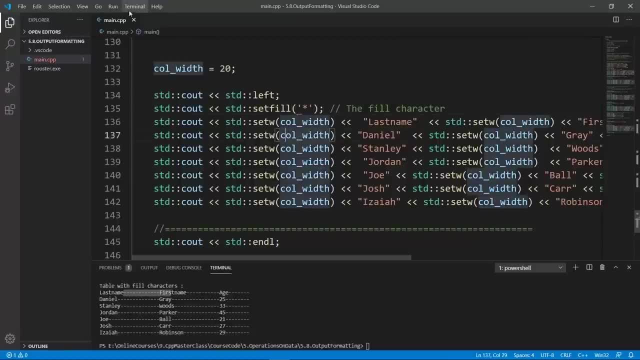 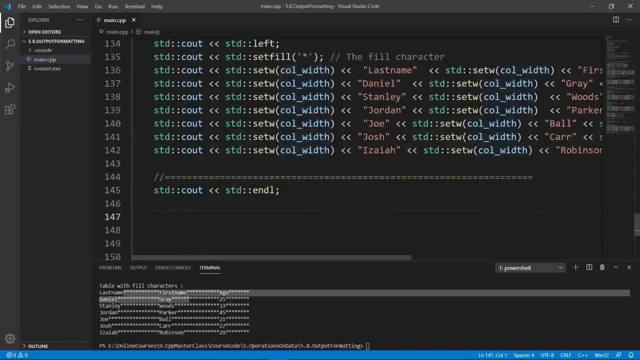 change this to a star. let's do that and i can build again. if i run this, it's going to be filled with stars right now. the next thing we're going to look at is std bull alpha. we have seen this before, but what it's really going to do is force the output. 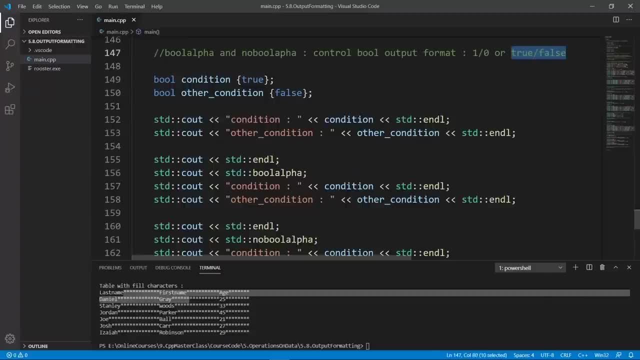 to be in the format of true and false, and the default is in the form of one and zero. here we have a few variables and they are of bull type. the first set of stdc out statements here is going to print in the format of one and zero, and then we're going to print in the format of one and zero. 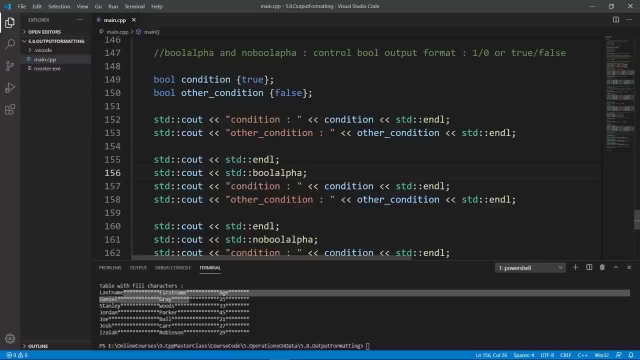 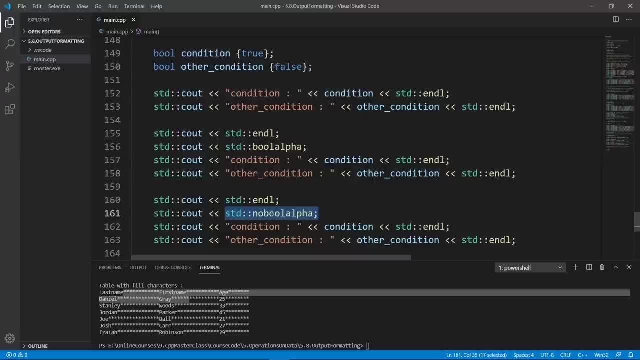 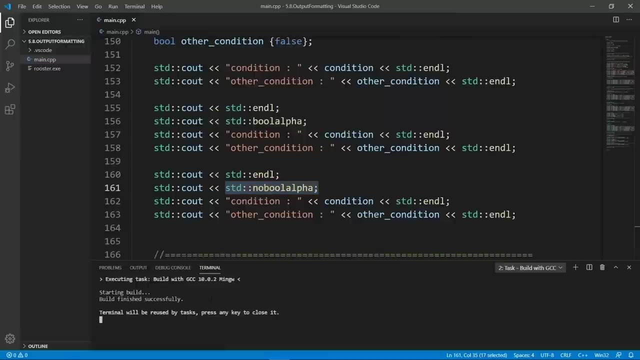 we are going to set the output to bull alpha and it is going to be in the format of true and false and we can disable the bull alpha. with this setting here, which says: std- no bull alpha, we can build this and see the effect of this. so we're going to run rooster again and you're going. 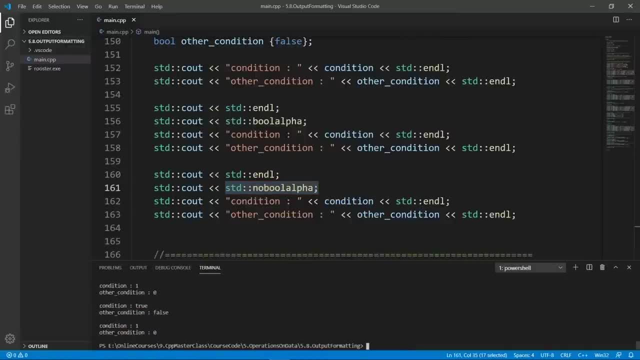 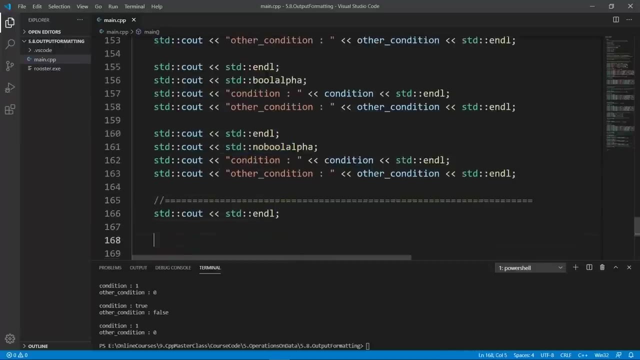 to see that condition one zero. condition true: false. condition one: zero. we are able to modify how our boolean data is displayed on the console using these two settings here. use them if they make sense for your application. the next thing we're going to look at is show pose and we're going to just put in the 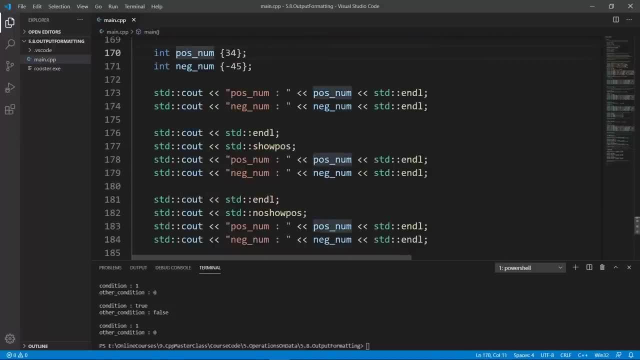 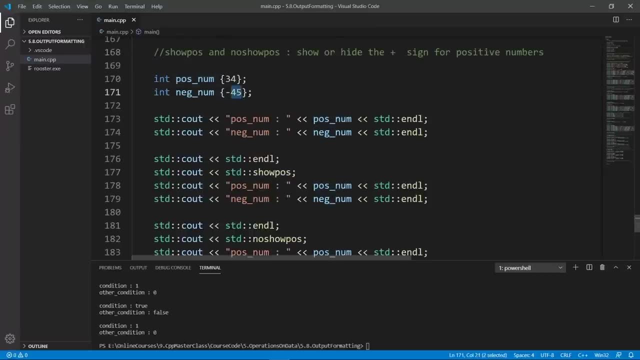 data. we have two numbers: positive number, which is 34, a negative number, which is minus 45, and we can decide if we want to show the plus sign for positive numbers. by default, the plus sign is going to be hidden. it's not going to be shown if you want it. show the plus sign for positive numbers. 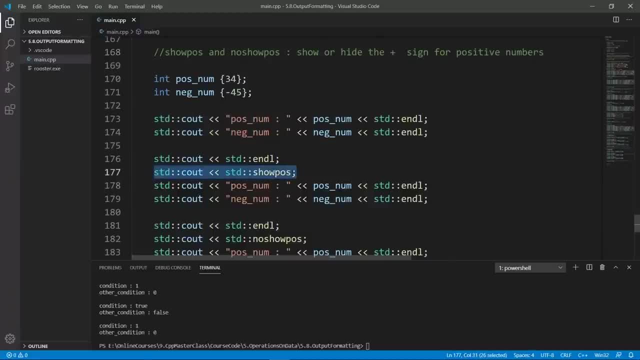 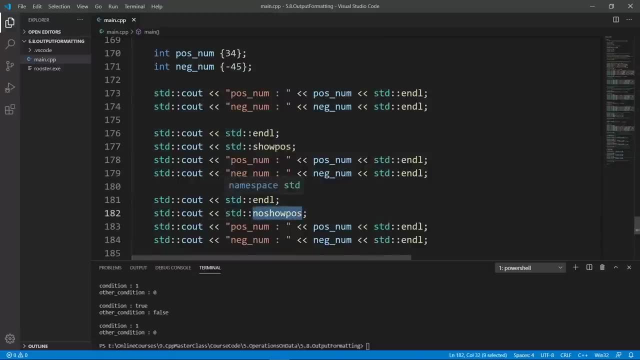 you can use the show pose manipulator and if you want to disable that when it was enabled, you can use no show pose and this is going to do what you want. we can build this again and if we look at the output, we're going to see that pose num doesn't have a plus sign in front because, by default, the 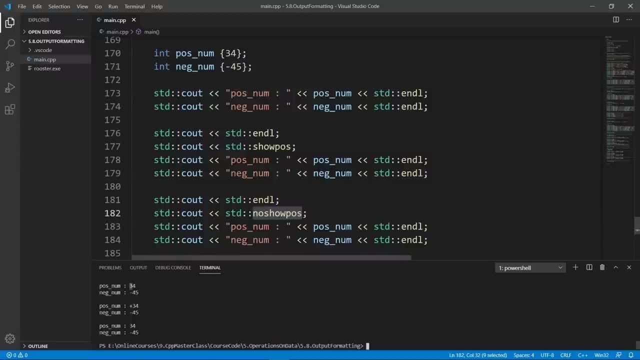 show pose is disabled and we set the setting here and we're going to see the plus sign and if we disable that, we're not going to see the plus sign and if we disable that, we're not going to see the plus sign again. this is the effect of std show pose and std no show pose manipulators. we can also. 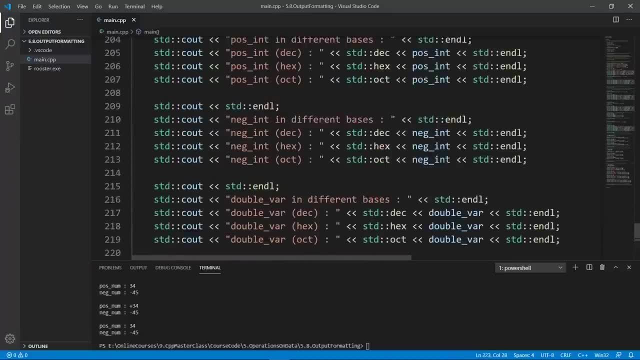 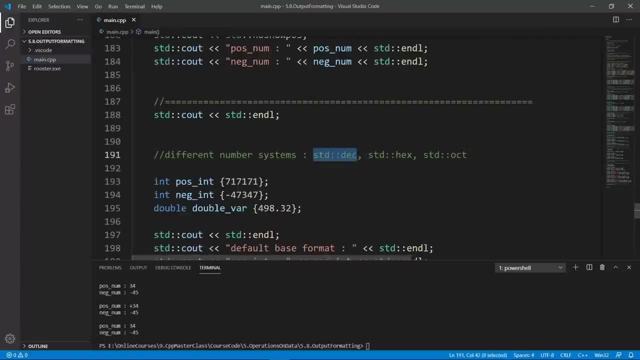 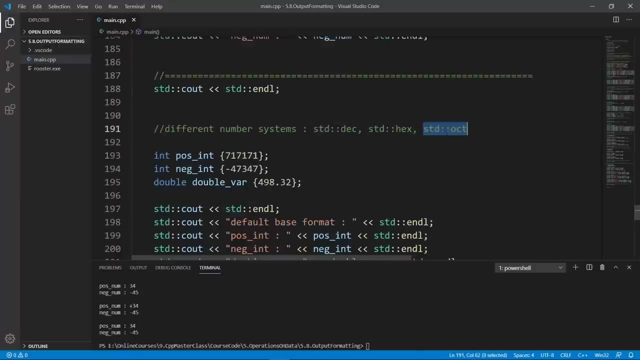 affect the base in which the data is displayed on the terminal, and we do this by setting the output base system. we can set std deck to force the output in decimal, std heads to force the output to be in hexadecimal and std oct to force the output in octal and. 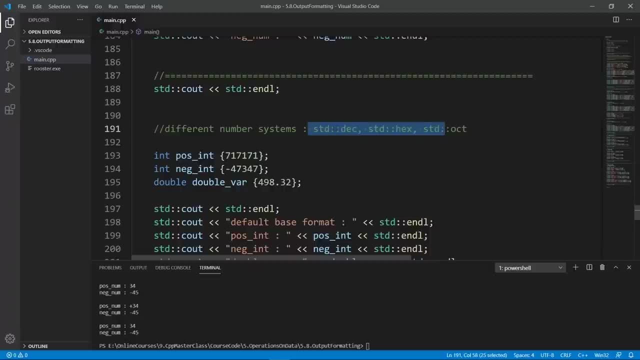 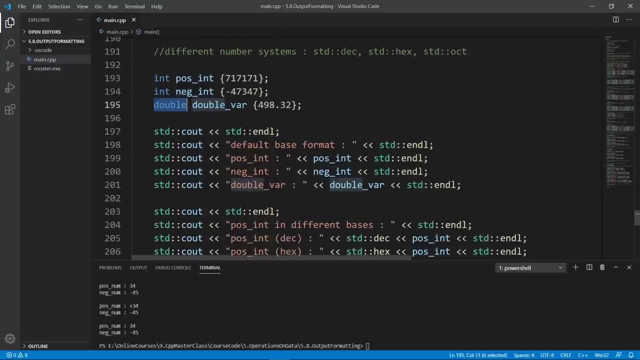 this is only to take effect for integral types. this is not going to have effect for floating point numbers, for example. here we have a few variables, a positive integer and negative integer, and a floating point number which is the double, and we're going to try and print these things. 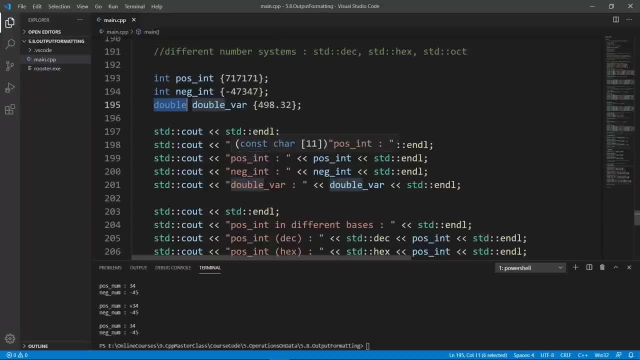 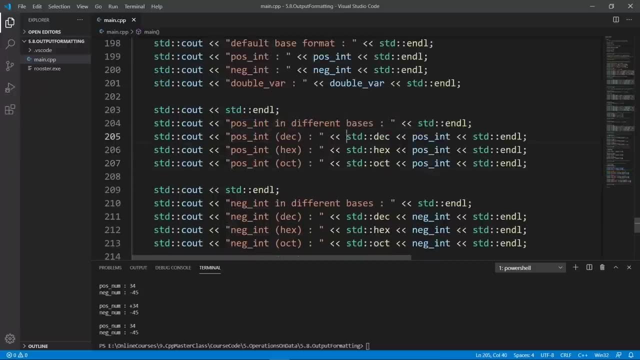 in all these base systems. we're going to print these things in the default format. we're going to see how they look. we are going to take the positive number and show that in these different number systems. we're going to do the same for the negative number and we're going to show that. 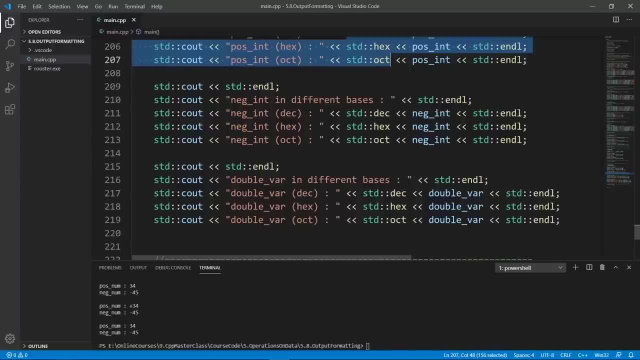 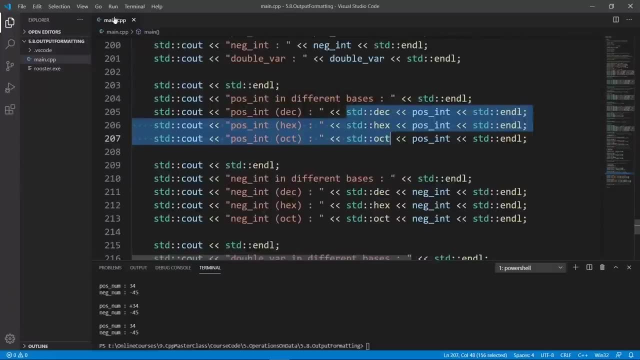 this doesn't have effect on floating point numbers, because these number systems don't really work for floating points. we can run this and see the output. we are going to run the task that is going to build with gcc and we're going to clear and run rooster and what we're going to. 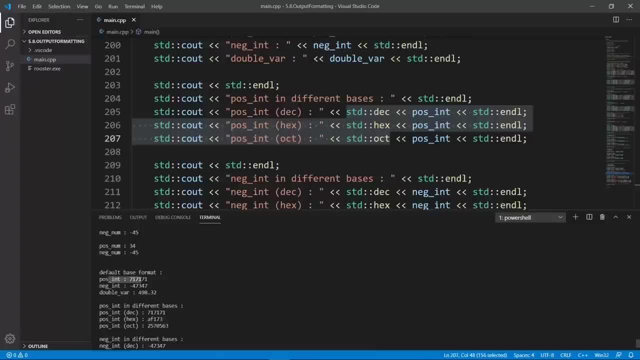 see is that, by default, positive number is going to be this, negative number is going to be this and our double var is going to be this and we are going to take the positive number. show it in different base systems. in decimal it's going to be like this, in hex it's. 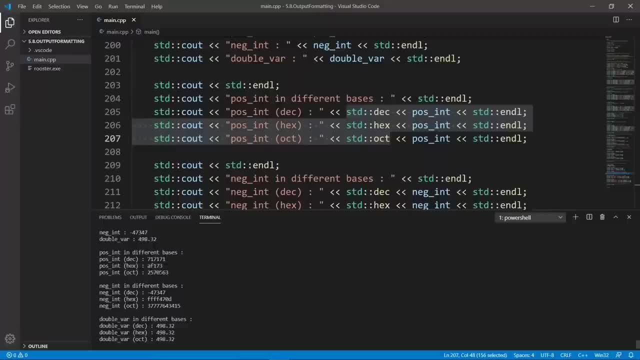 going to be like this. in oct, it's going to be like this: the negative number is also going to be in this format here. so if we show it in decimal, it's going to be like this: hex it's going to be like this, and octal it's going to be like this: you can see that the double var, which is a floating 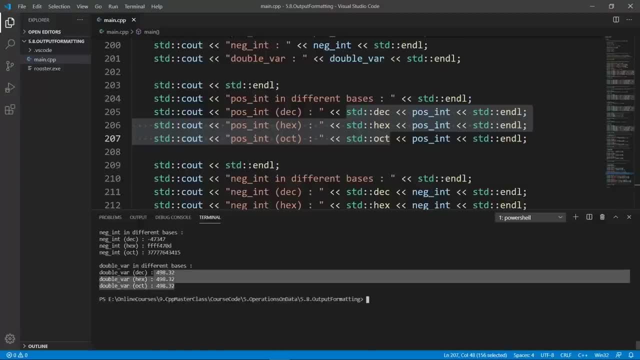 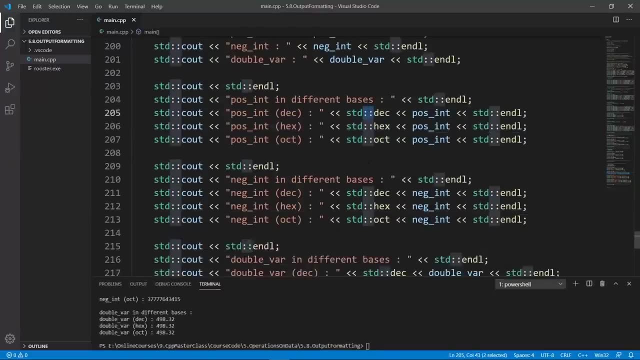 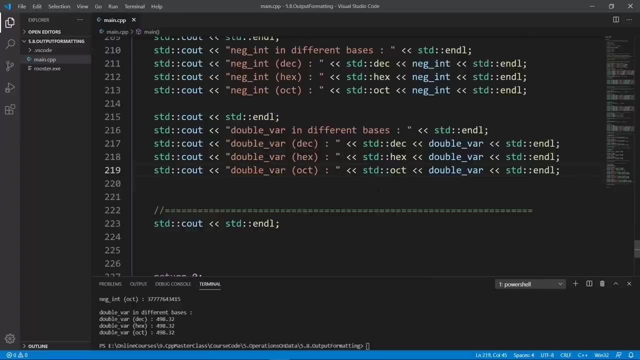 is not really affected. it's going to be showing in the same format, regardless of the base that we set here. one thing you should know is that this base setting here is going to stick. so here, for example, you see that we have set output to octal. so any other thing that we're going to print out. 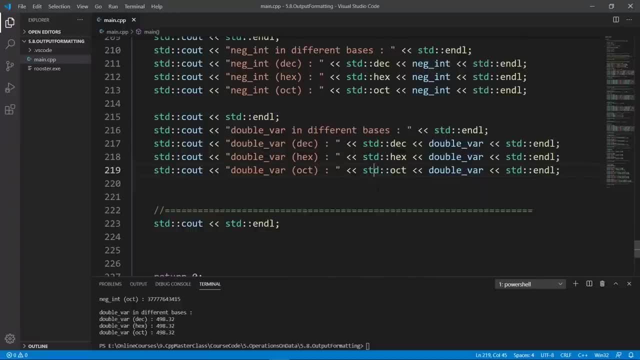 is going to be shown in octal and we have to be sure that's what we want. if that's not what we want, we will have to reset the output number system. it's going to take effect. this is how you can use these things to affect different number systems. 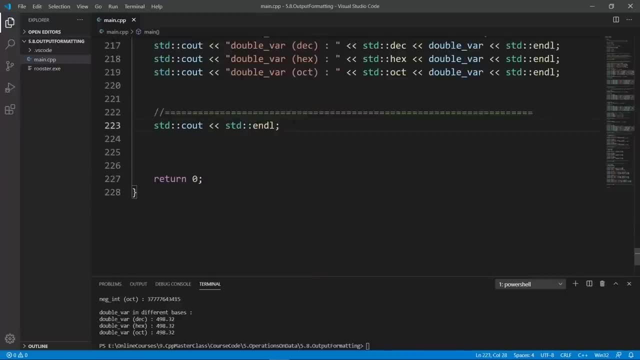 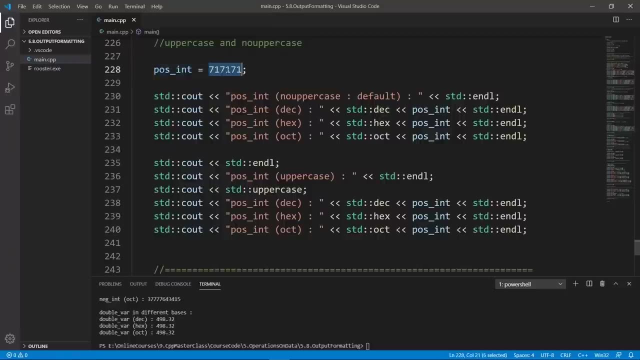 for output in your terminal. we have seen that you can also force things to show up in uppercase if that's important for your application. for example, here we have a positive number. if we show that in hex, this is going to contain a few characters, and if we don't set uppercase, it is going to show up. 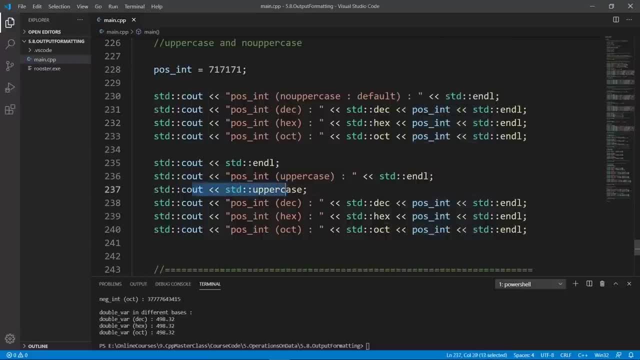 in lowercase and if we want it in uppercase, we can set this set in lowercase and if we want it in setting and it is going to show up in uppercase. this may be helpful in some applications and i just want you to be aware of these things. we're going to world and run our application. 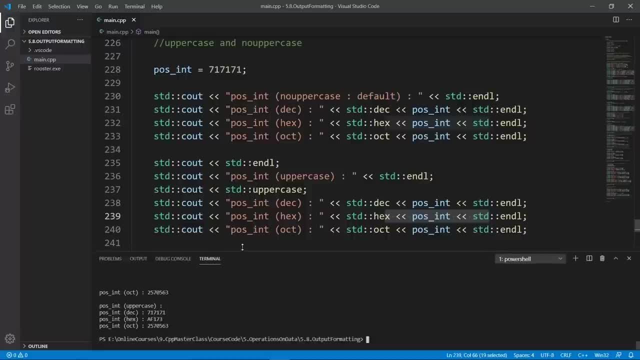 you're going to see that let's bring this up a little bit so that we have some breathing room. our positive integer here is going to show up in lowercase here in hex, because this is going to contain characters and if we set uppercase, you're going to see that it's going to show up in lowercase. 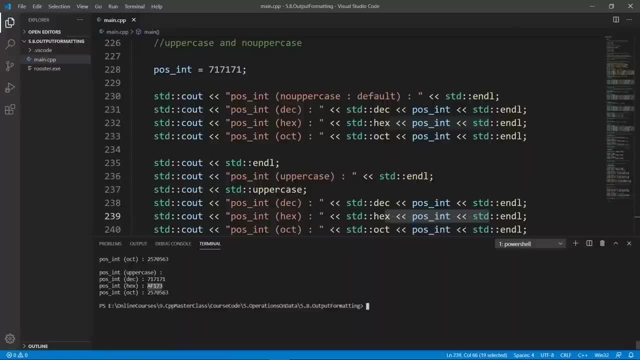 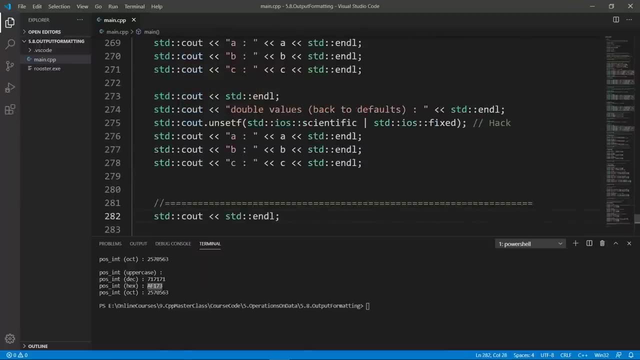 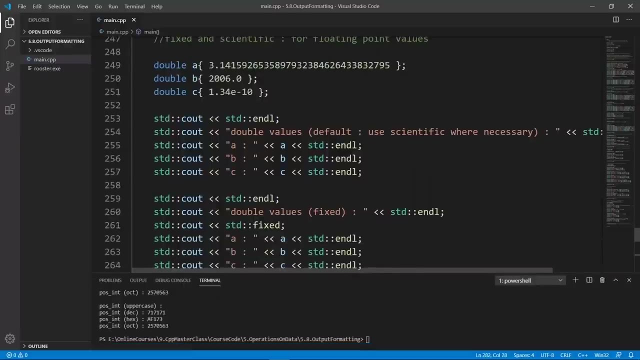 the characters are going to show up in uppercase and this is the effect of this setting. here we can also affect how floating point data is printed out on the terminal. for example, here we have a few variables- a, b and c- and by default they are going to show up with decimal points and use scientific 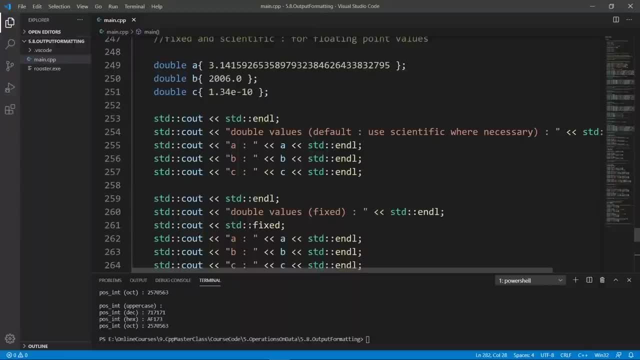 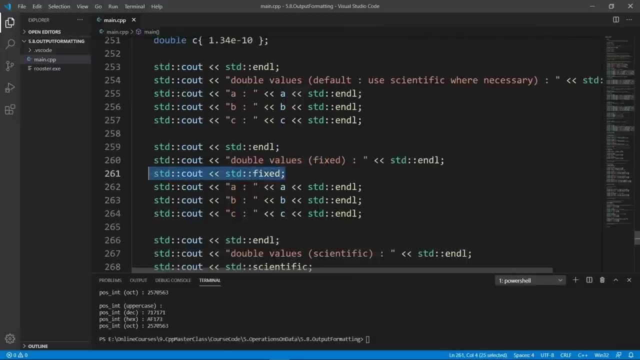 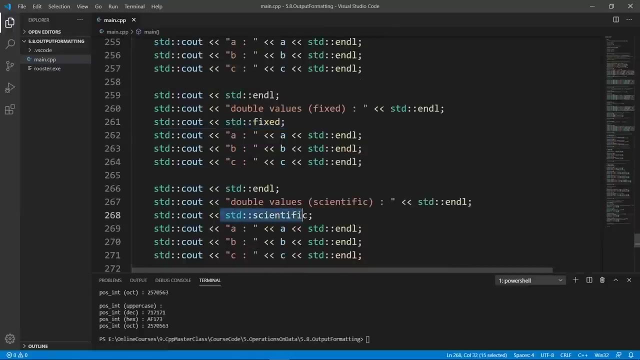 notation where necessary, but we can choose to use fixed, for example, if that's what you want. we need in our application and the output is going to be shown using fixed notation with decimal points. if we want, we can force the scientific format and we do it like this and all output is. 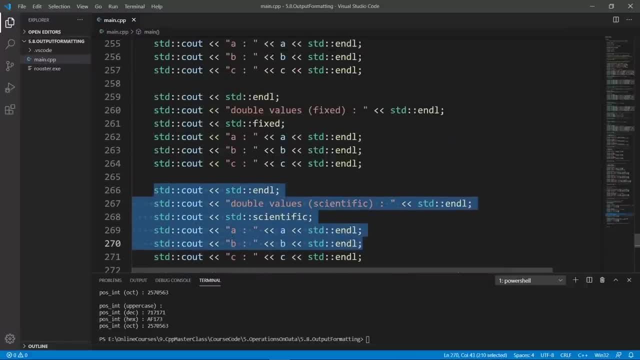 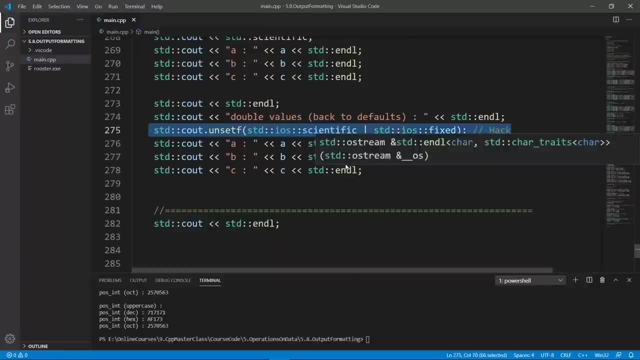 going to be in scientific format and we can disable all these settings and reset this to the defaults with this piece of command here. there is no official way to set floating point output to the defaults, and this is a hack i actually learned about when i was preparing the code for this course. 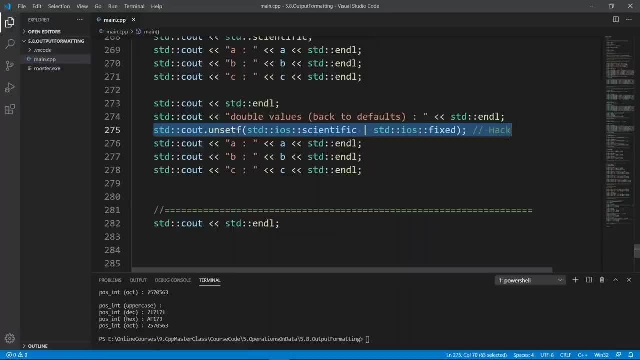 and the proper explanations for this are really out of scope for this course. so if you want to reset the floating point output format to the default, you're going to use this, but we don't really have enough tools to understand this yet. so just take it by faith and 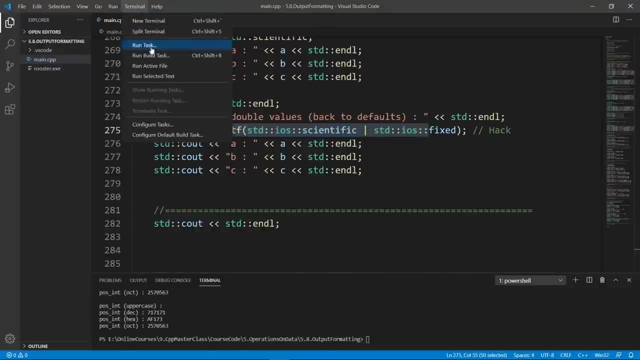 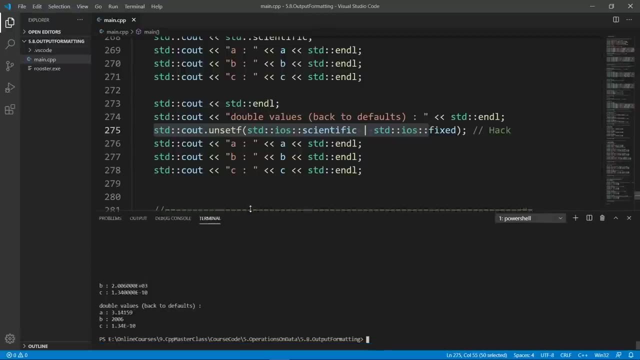 you're going to see that if we run this, it's going to work. let's try and run this through the compiler and the world is going to go through. if we run this and bring this up a little bit so that we have a little bit of breathing room, we're going to see that our double values are a, b and c. 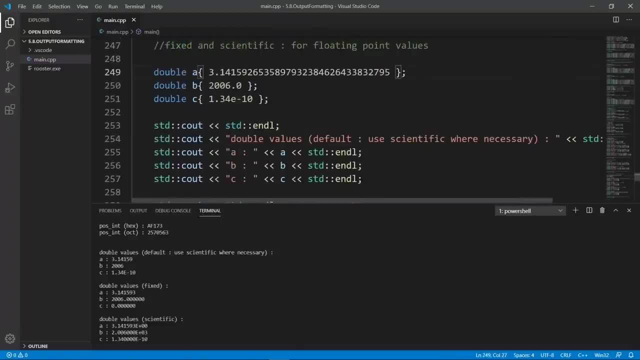 and that's what we have in our code here, and by default it's not going to be able to show these things because of the precision limits. so we're going to have 3.14159. it's going to go up to here and the rest is going to be chopped off if we use 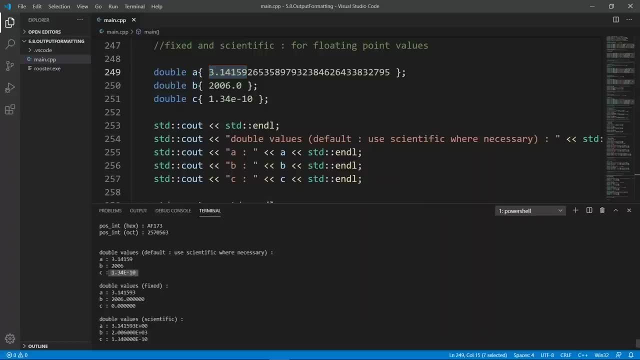 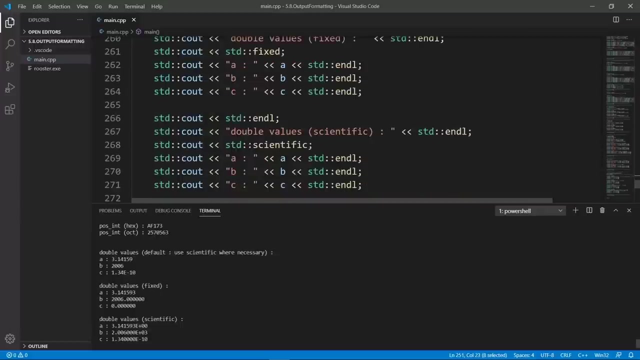 fixed format. you're going to see that whatever we had in a scientific format, it's going to show up in fixed format. and again, this is a really low number. that's why we have 0.0000 here. we can force the output to be scientific, as we did right here, and all output is going to be. 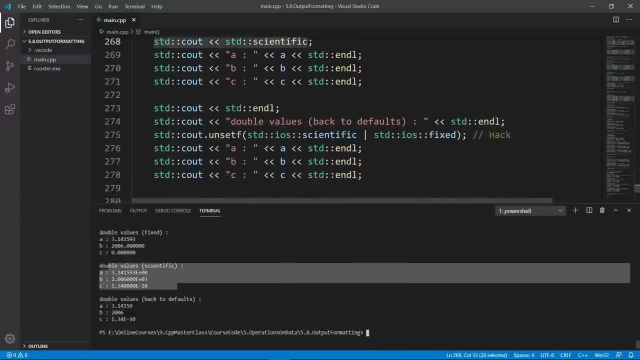 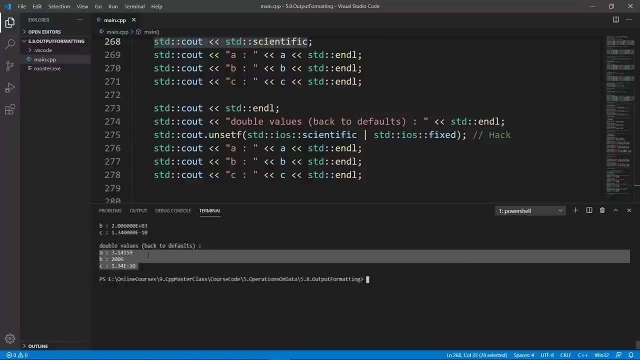 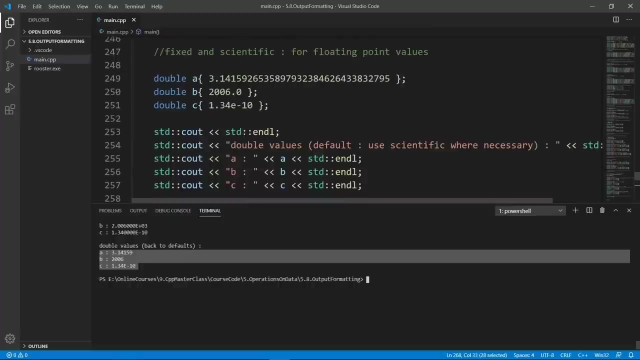 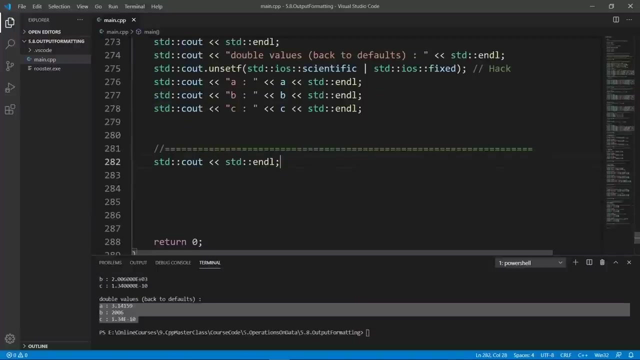 in scientific format. down below. here we use our hack to set to the defaults and you see that it's going to go back to the initial format that we had before. this is how you use std fixed and std scientific to manipulate how your floating point numbers are printed to the terminal. we have also 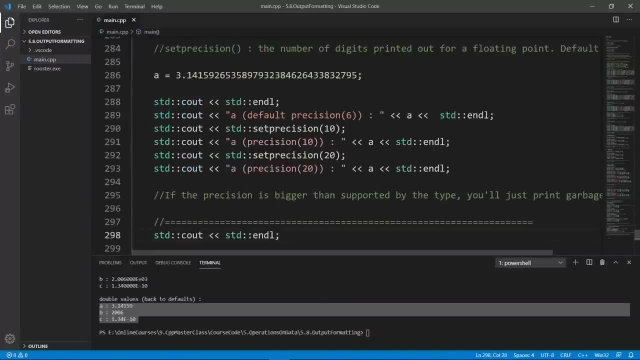 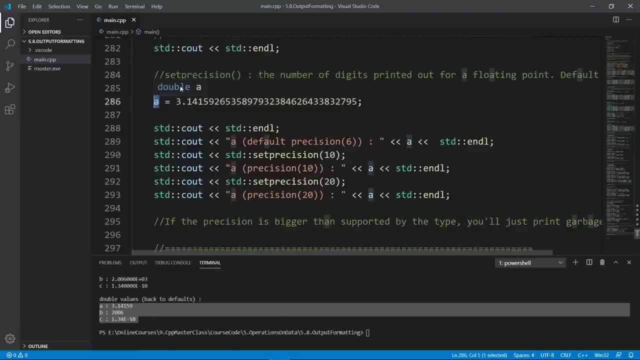 seen that we can set the precision of our output in the terminal. you can also see that we can set the precision of our output in the terminal. we have also seen that we can set the precision of our output in the terminal. here we have a variable a. it is of type double, as you can see in a visual studio code here. if 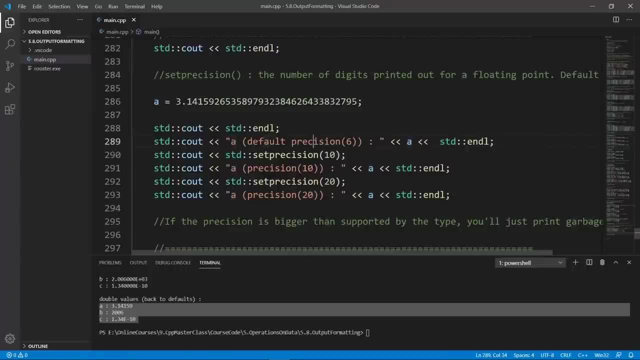 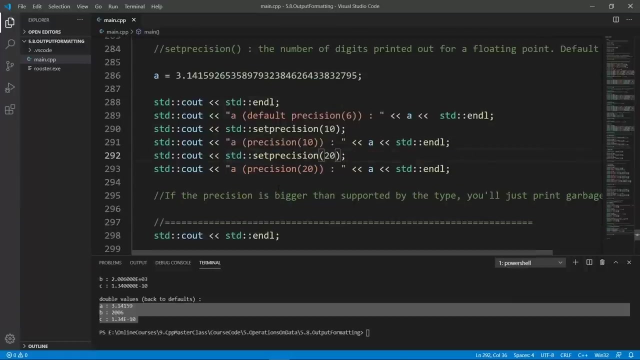 you hover over a variable, you're going to be able to see its type. we can choose to see this in whatever precision we want. 6 is the default in our case here, but we can choose to set the precision to 10, 20 or whatever it is really we want. please note that this is going to be limited by the. 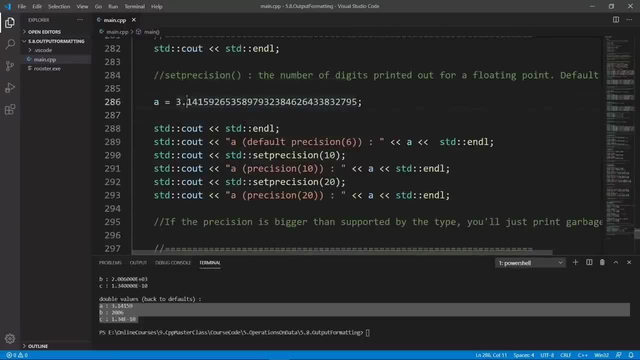 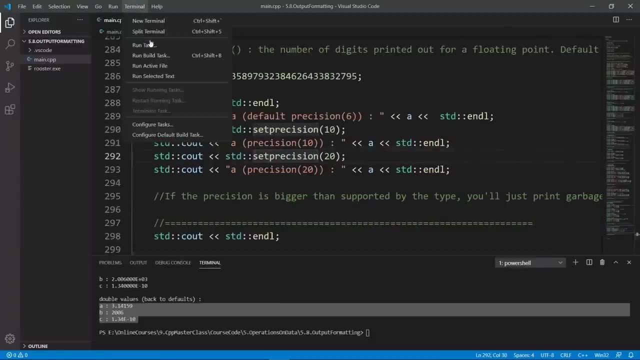 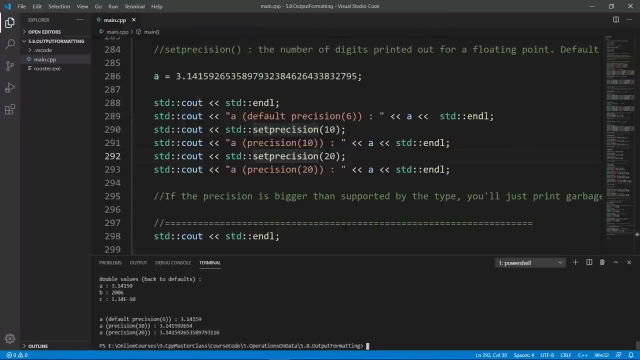 number of digits we are going to use. the double has a precision of 15 and if we have more than 15 digits in here, the rest is going to be garbage. just be aware of that. we're going to try and build this and we're going to use gcc as usual, and if we run this, we're going to get our numbers in. 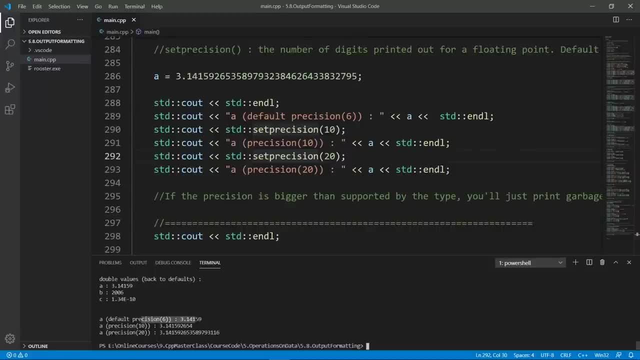 different precisions. the first one is using the default, which is going to be sex. if we use 10, we're going to get 10 digits. if we use 20, we're going to get 20 digits. but if we go all the way over the precision that our type here supports, we're going to get garbage. i hope this makes sense. 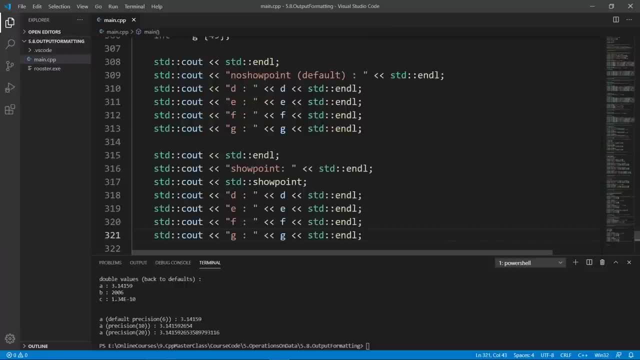 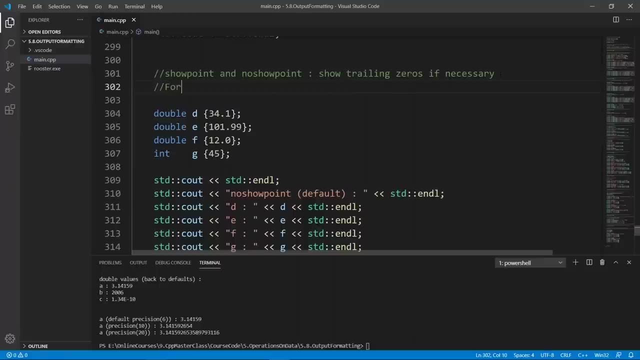 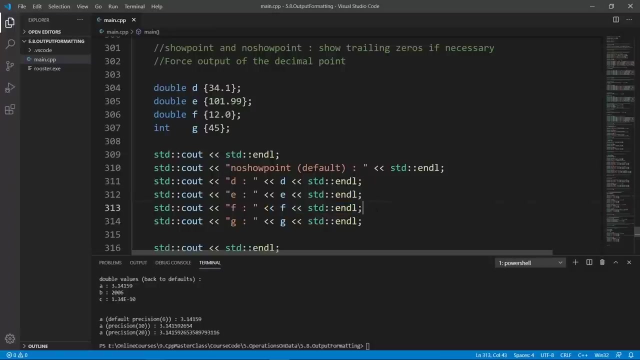 the last thing we're going to see is show point, and we have seen that this is used to force outputting the decimal point. let's say that here, and a good example for that is this 12 here. if we print it out here, we're not going to get the decimal point by default, it's going to print 12. 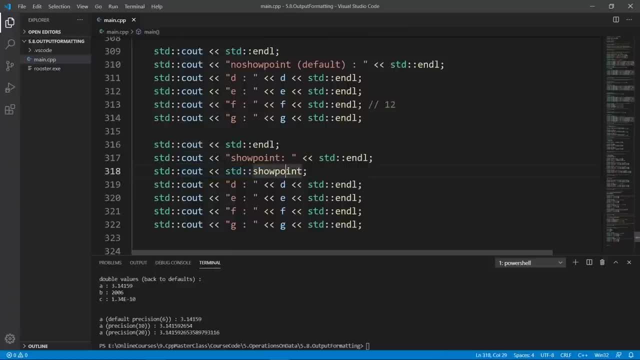 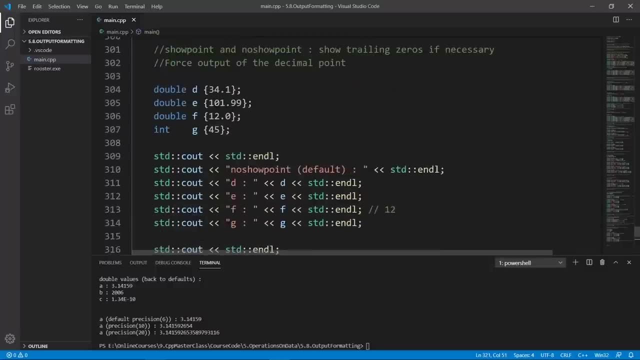 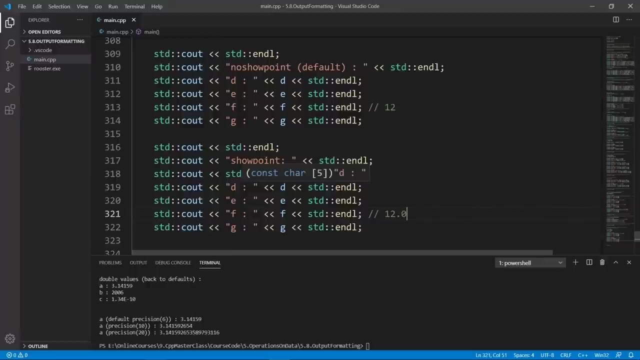 but if we go down and force output of the decimal point here, we're going to get something like 12.0, and another effect of this is that it's going to add trailing zeros to fill whatever space is allocated for your output variable in the terminal. let's try and run this so that we can actually see this. 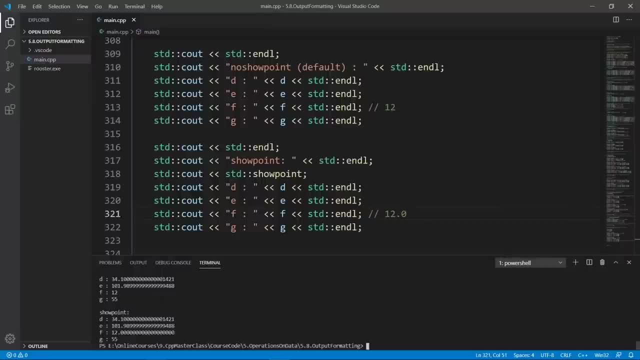 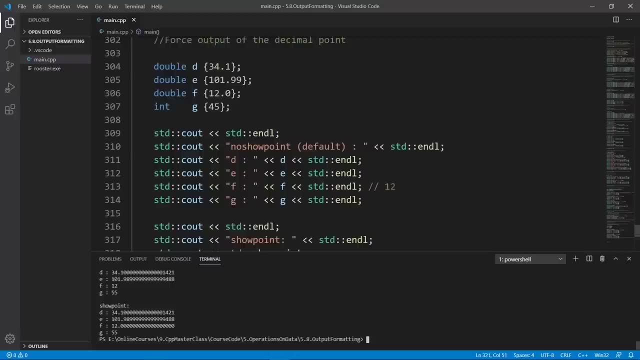 running. we're going to run our rooster executable and in the first group here we don't have the settings for show point. and if you look at the numbers that we had in our code, the first number is 34.1 and you see that we are padding a lot of numbers because we had set our precision to a really big 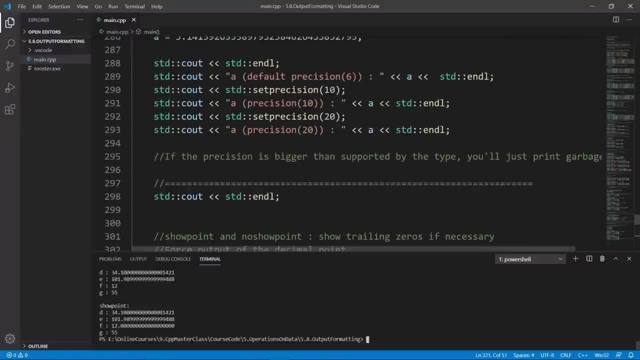 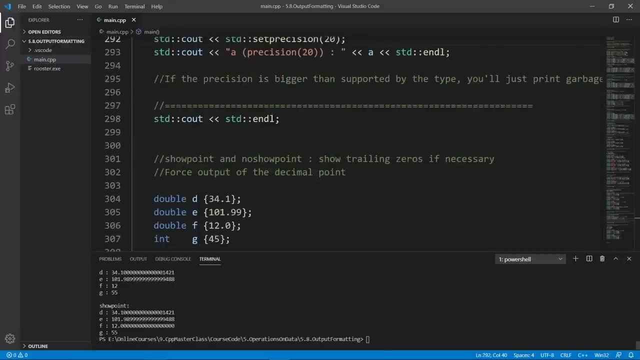 number in the last example that we have run. let's actually go there and show you that. that's why we're seeing the precision of 20. it is really huge but no big deal. we can reset this to whatever we want if this is too much for us. the important thing here is that we can set the precision to. 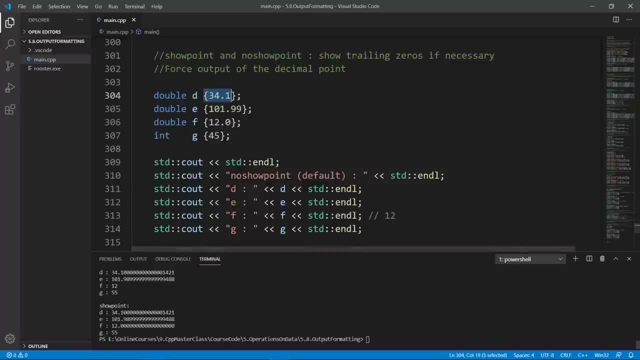 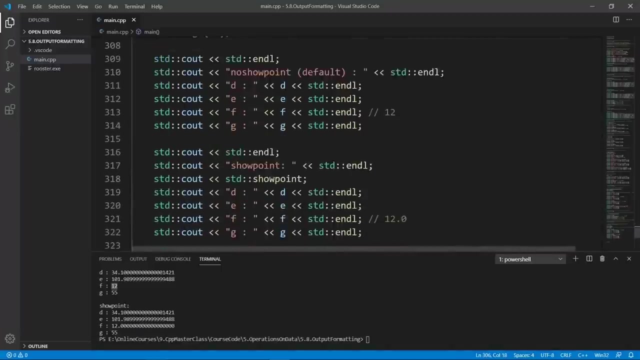 30.1 and that's what we are seeing. and if you go to our 12 here, so you see we have 12.0, but our output is not showing the decimal point here. if it is important to show the decimal point, we can do. 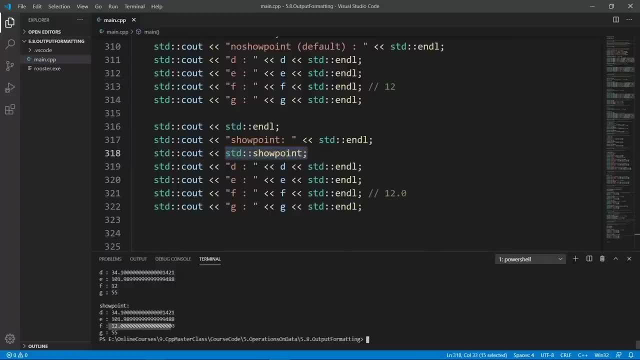 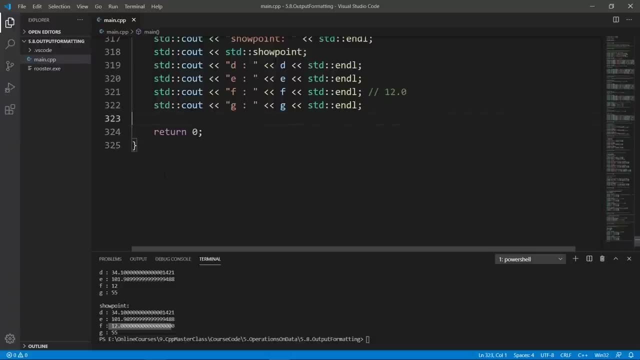 std show point here and it is going to show up. this is really what is important in this piece of code here, and this is really all we set out to do in this lecture. we had a chance to play with a lot of code here, and we're going to show you how to do that in this lecture, so let's go. 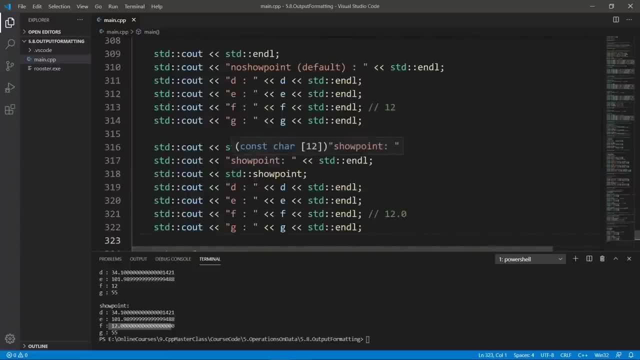 ahead and we're going to play with a lot of these manipulators and the best way to learn about these things is really to try them out in code and try to change a few things and see how that affects the output you get in the terminal, and we had a chance to play with many of these things in this. 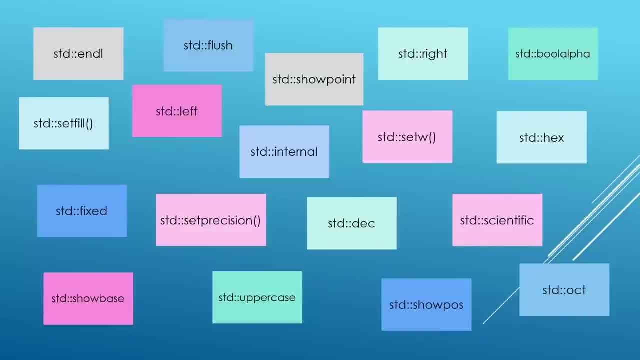 lecture. there is a lot of these guys. i tried to make this lecture as extensive as i can. that's why it turned out to be pretty long, but once you've learned about these things and played with them in code, you're going to be able to play with a lot of these things and you're going to be able to. 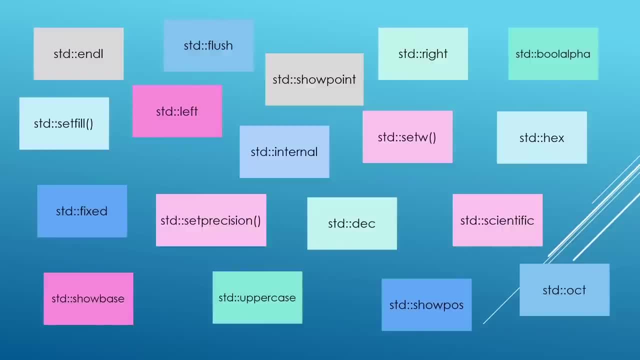 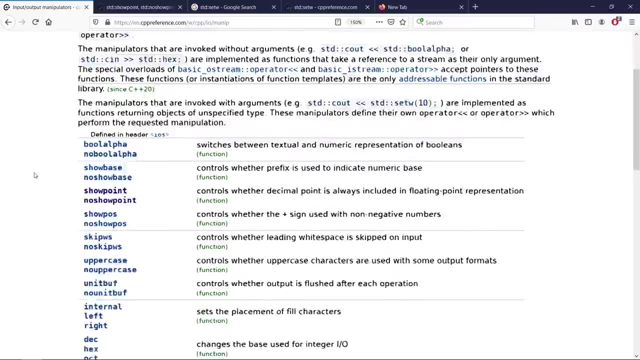 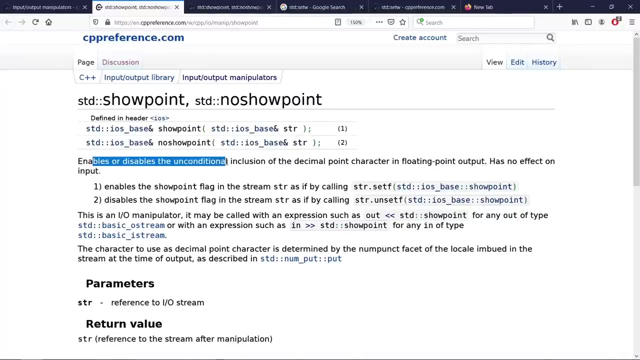 use them in code. you're never going to forget them. one last point i want to emphasize again is that the documentation is of utmost importance. it is really good to come here and check things out. for example, if we go to show point here, we are going to get a nice explanation of what this. 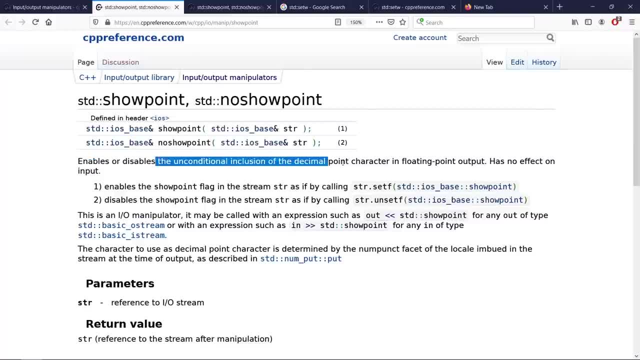 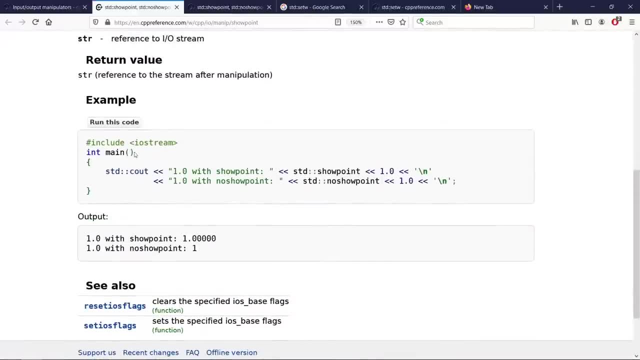 manipulator does, enables or disables the unconditional inclusion of the decimal point character. and you can read all this and the nice thing is that if you go down, you're going to get a piece of code that you can use to really understand whatever it is they are talking about. 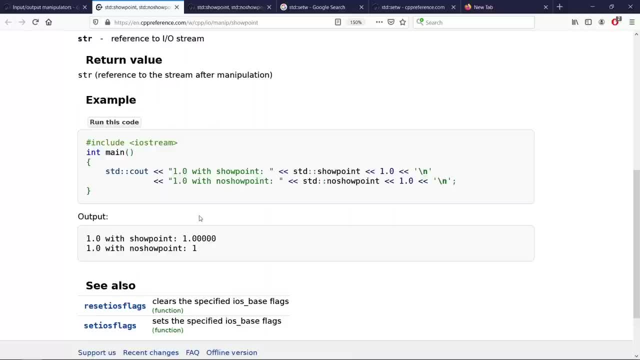 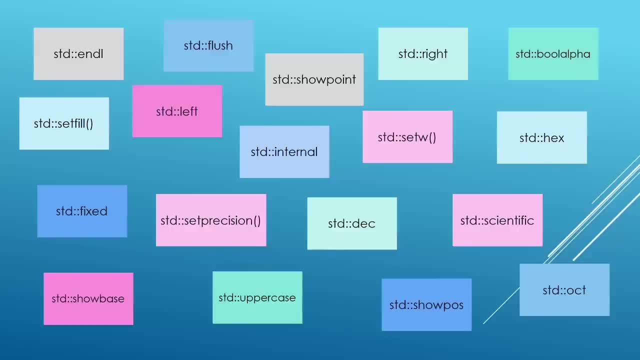 and this is priceless. if you are learning, it is a good thing to be able to use the documentation. this is really all we set out to do in this lecture. it turned out to be really long, but i really hope it was worth it for you. we're going to stop here in this lecture. in the next one we're 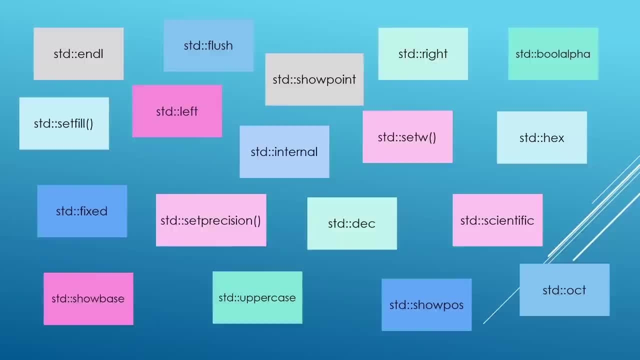 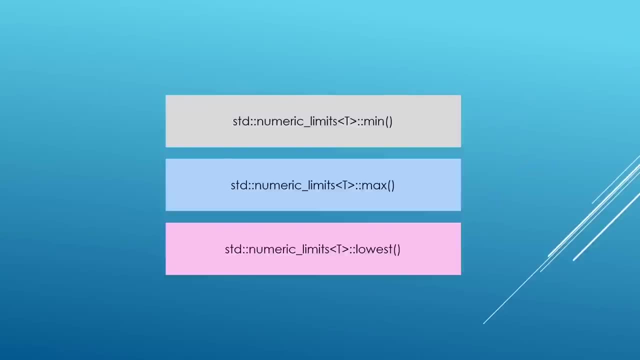 going to learn about numeric limits. go ahead and finish up here and meet me there. in this lecture, we're going to be playing with a few functions from this library. specifically, we're going to be looking at the minimum, the maximum and at the lowest functions, and this is really. 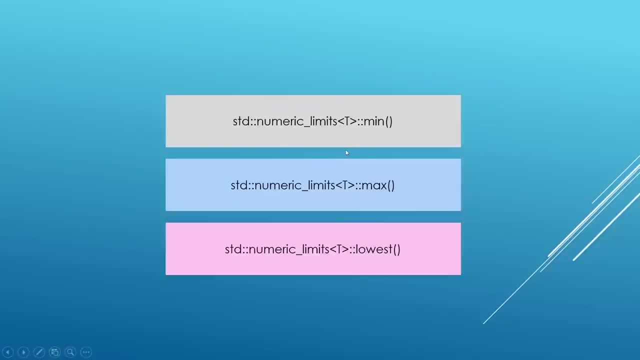 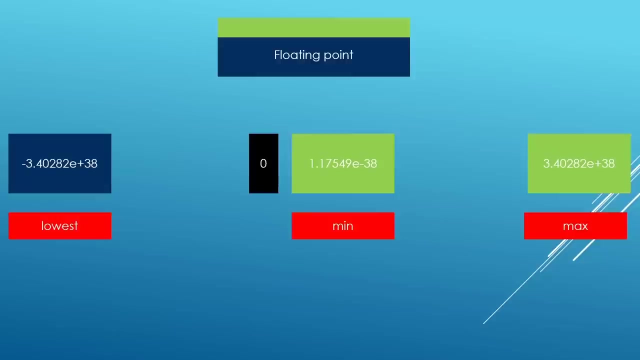 how you use them. you can think of this t as a placeholder for the type for which you want to know the minimum, the maximum and the lowest point respectively. i know this might be cryptic to some of you, so we're going to look at a few specific examples here. we have a simple 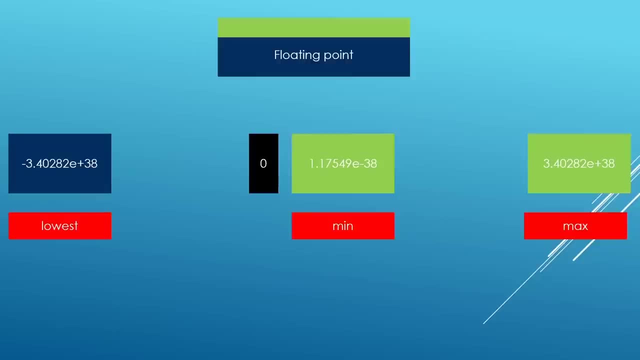 explanation of what these functions mean for floating point values. the minimum is going to represent the smallest positive number that is representable with that floating point type. the maximum is going to be the maximum floating point number you can represent and at the lowest number is going to be the lowest negative number you can represent. with that type, things change a little bit. 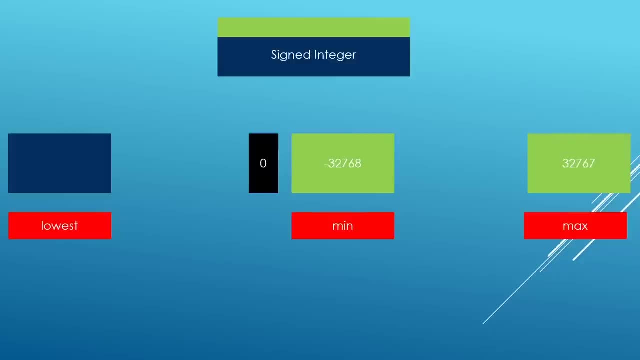 when you start dealing with integers and this, functions are going to look like this: the minimum is going to be the minimum number you can represent with that integer, and lowest doesn't really mean anything for integral types. the maximum is going to be the maximum number. one thing you have to keep in mind is that the minimum may be negative. 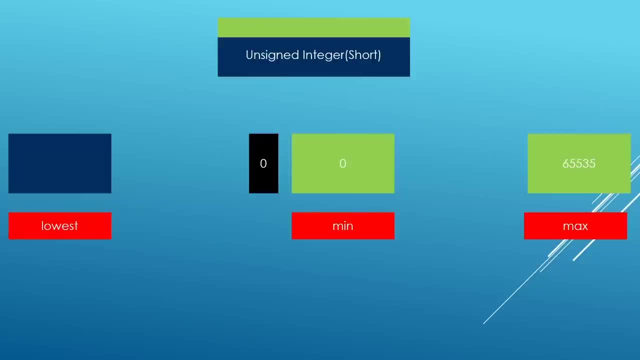 if you are using a signed integer. if you are using an unsigned integer, for example for short, minimum is going to be zero and maximum is going to be the maximum number presentable with that integer type. here we are looking at numbers for short end, but the same 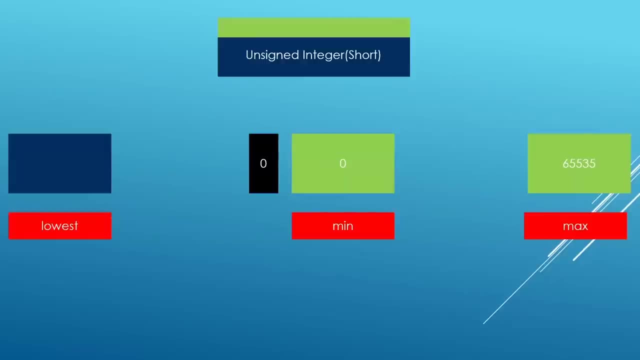 story applies to whatever integer type you are using, even if you happen to be using long, end or end without any modifier. remember that we had to do a lot of things to get this range, and it was really hard to even do this for floating point types, so this library is helpful. 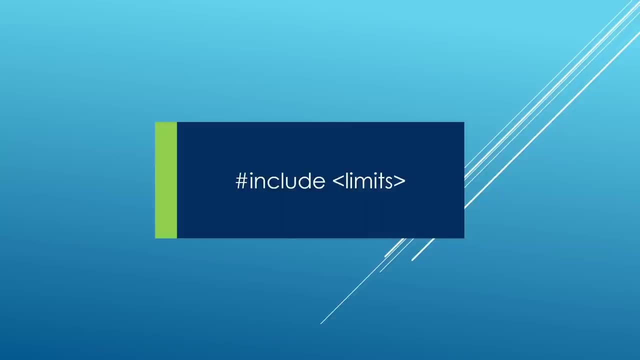 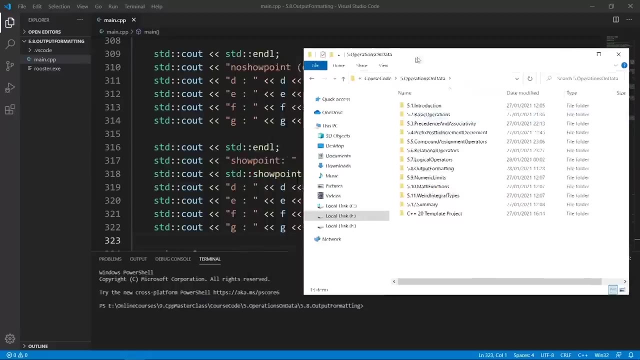 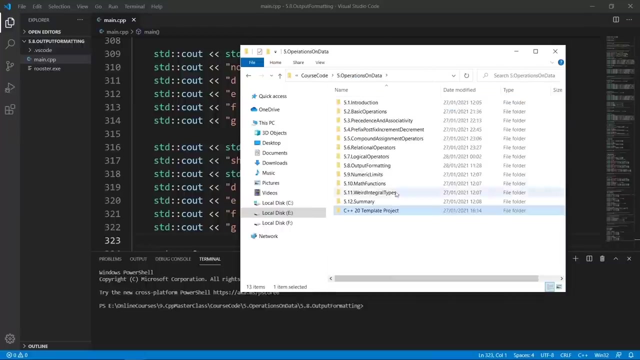 in getting a sense of what we can represent with the given type, be it floating point or integral. let's head to visual studio code and play with us. here we are in our working folder, we are going to copy code from our template project and we are going to go in the current. 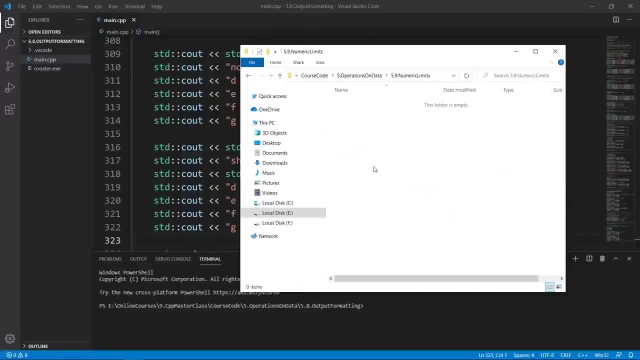 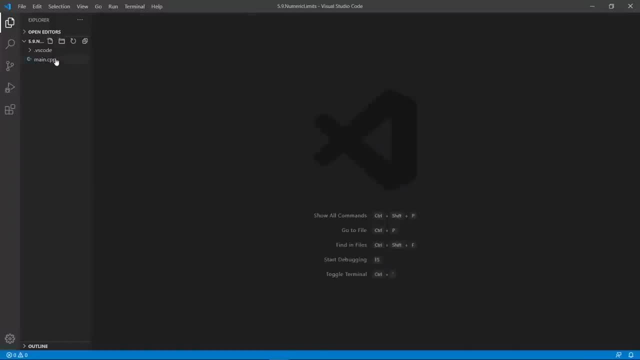 project, which is numeric limits. we're going to go in, put in our files, go up again and open this file up in visual studio code. we're going to close this up, open the main cpp file, remove whatever it is we don't need. we are going to include the limits library. 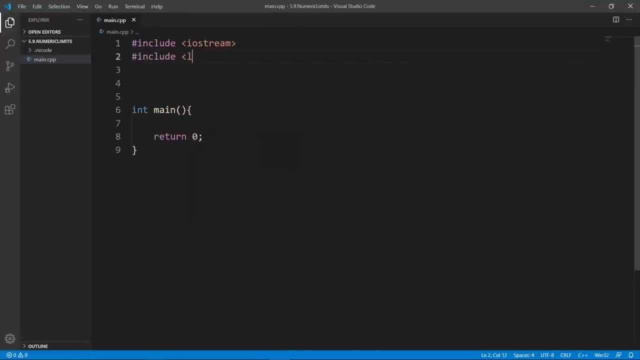 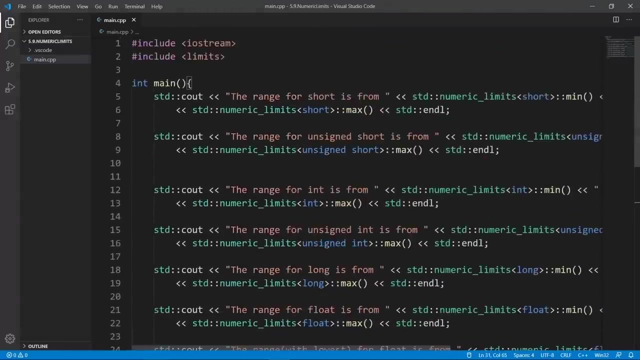 remember. this is the first thing we need to do if we want to play with these facilities that we just looked at in the slides and we are going to go down here and put in the code we want to play with, and it is ridiculously simple if you have watched the slides. we just did in a minute, so what we're? 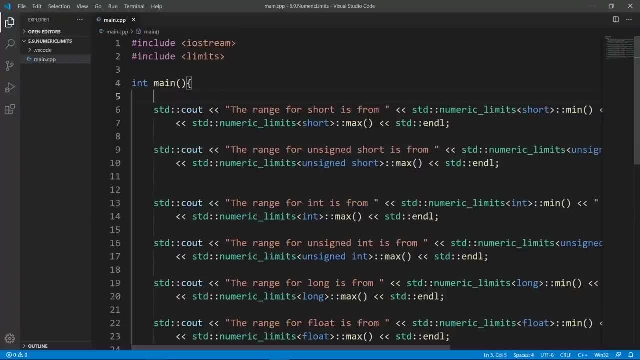 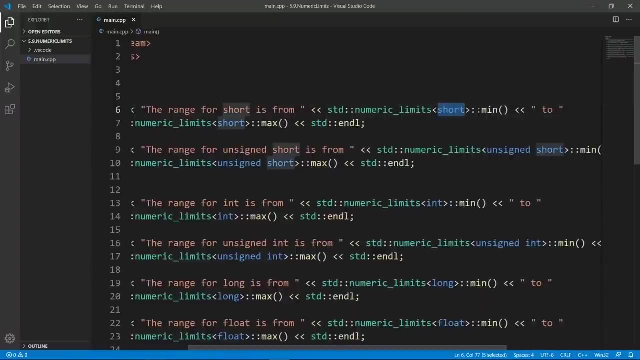 going to be doing here? we're going to be printing out the range for each possible type we want to play with here. so we're going to say the range for shoot and is from, and we're going to say std, numeric limits, short. that's what we want to deal with now and we're going to call the minimum. 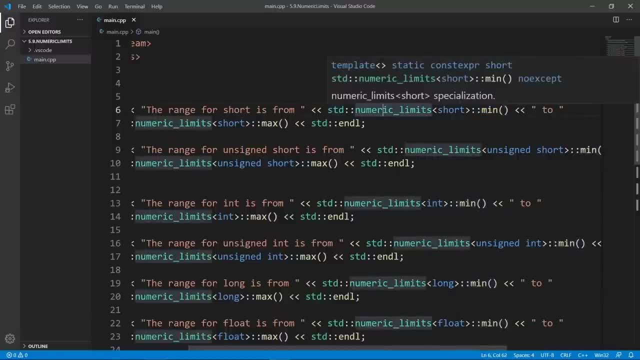 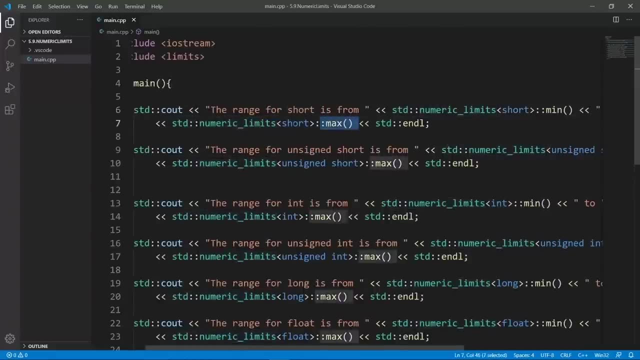 function. this is going to give us the minimum value we can represent with short and we're going to say std numeric limits and we're going to call the max function passing in the type for which we want to get the range for. and the same story applies for unsigned. 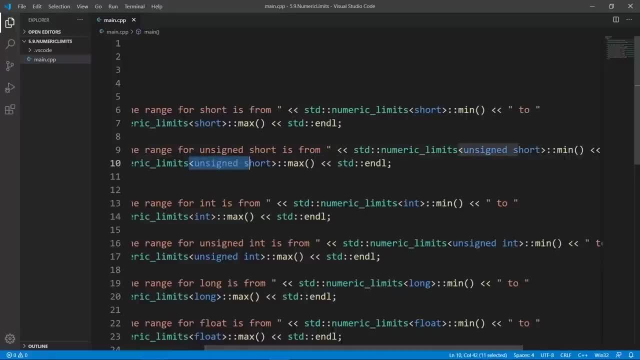 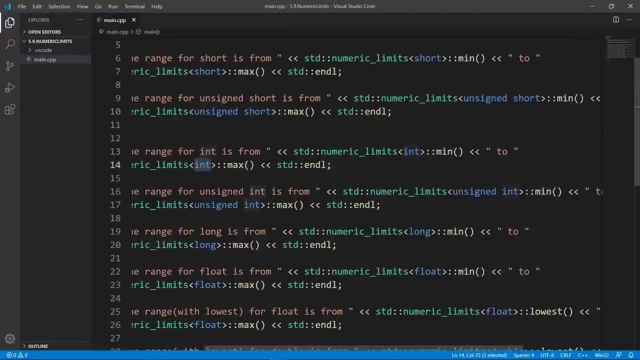 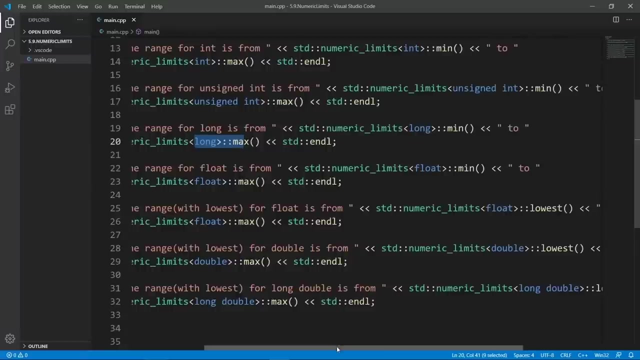 short. you see, that's the type we are using here. we are also going to play with int getting the range. we're going to use unsigned int to see how these things behave. we're going to use long and get the range, and we are also going to be playing with floating point types. so we're going 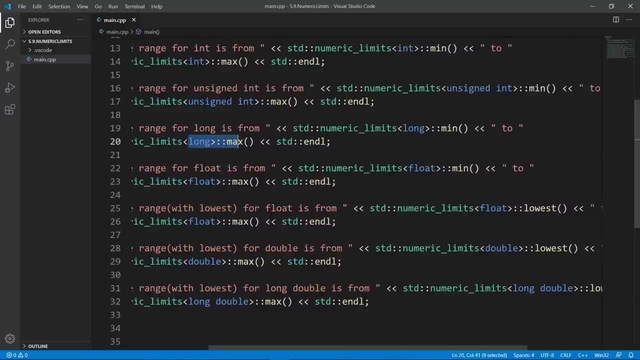 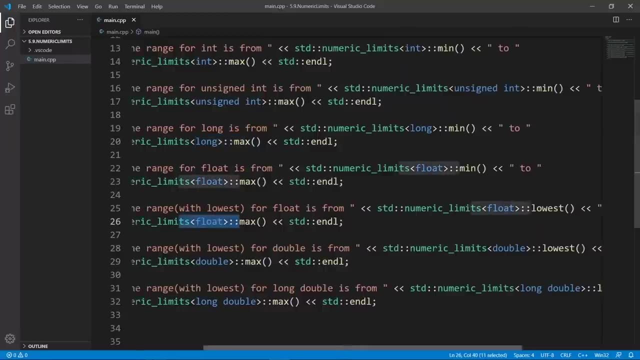 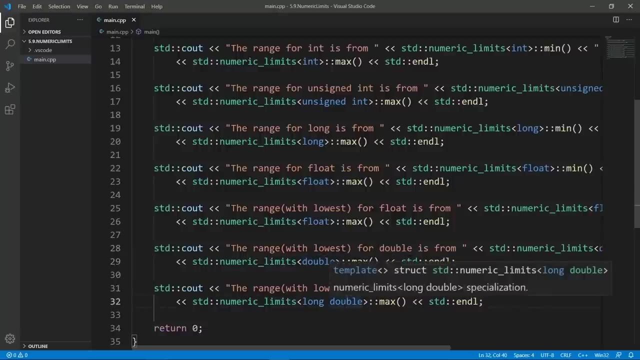 to compute the range using the minimum function and the maximum function, and we are going to be also using the lowest function to see that this really is the same thing we described in the slides. we're going to do this for double and long double and see how these ranges come up in this. 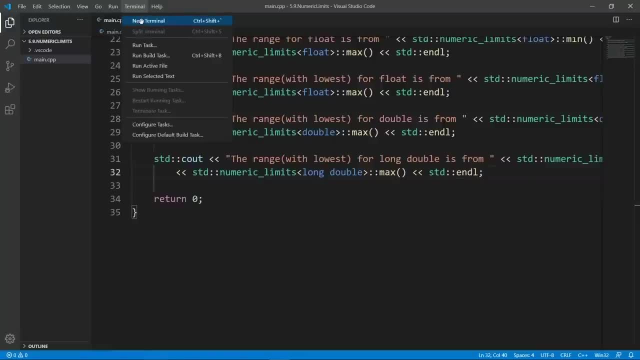 program. what we're going to do is open up a terminal. here we are going to run the test to build with gcc and the build is going to be good. you can go down and run rooster and we're going to get our values here. the range for short int is: 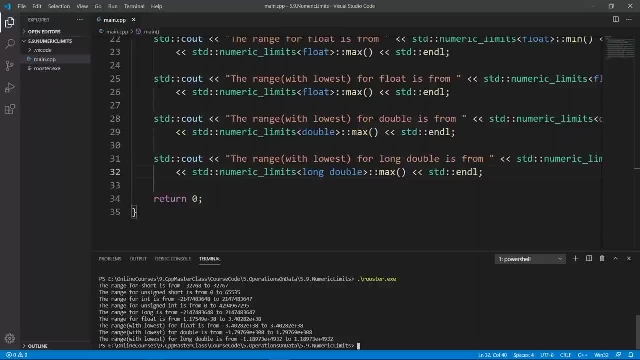 from minus 32, 7, 6, 8 up to 32, 7, 6, 7, and you see that this is exactly the same thing we saw in the lecture where we talked about number systems. we saw a way you can do this manually by plugging the. 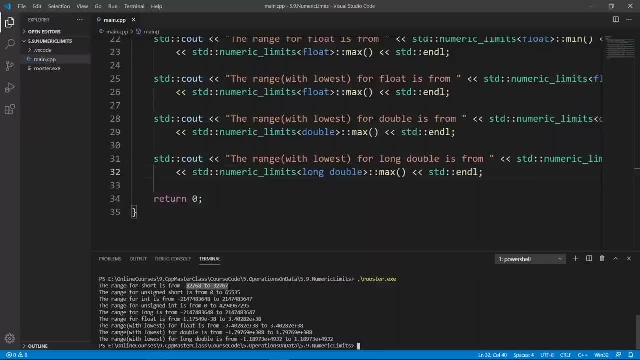 number of digits in some formula that we came up. you can go back and check that out if you want. we do the same for unsigned and and then we look at floating point types. we're going to print the range for float and if we use the minimum function to get the start of the range, we're going to get the minimum positive number. 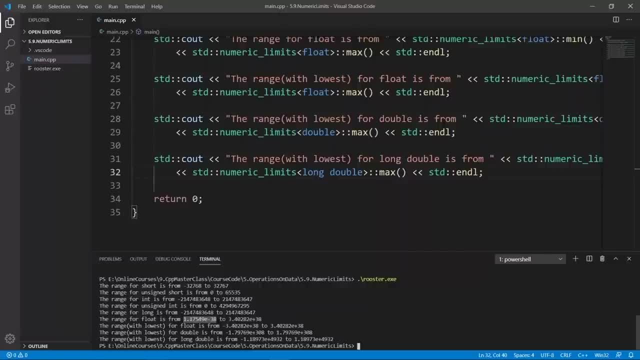 we can represent with a float. if we use lowest, we're going to get the lowest minimum number and then the maximum is going to be the same. if you think this is really small, you have the option to open up this folder in file explorer, or you know the computer environment folder or file explorer. 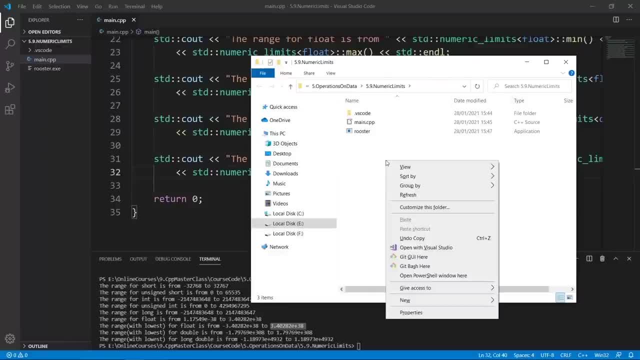 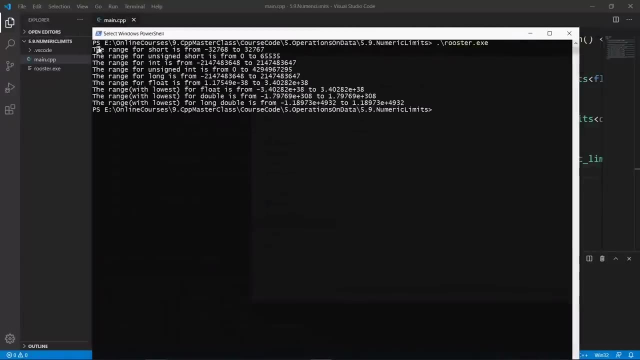 and you can open a command prompt or a PowerShell window by hitting shift and right-clicking and choosing this option here. open PowerShell window here and you're going to get a bigger window in which you can type things. We're going to run Rooster and we're going to see things in. 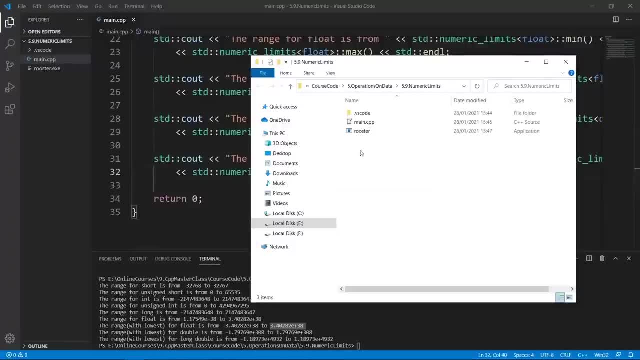 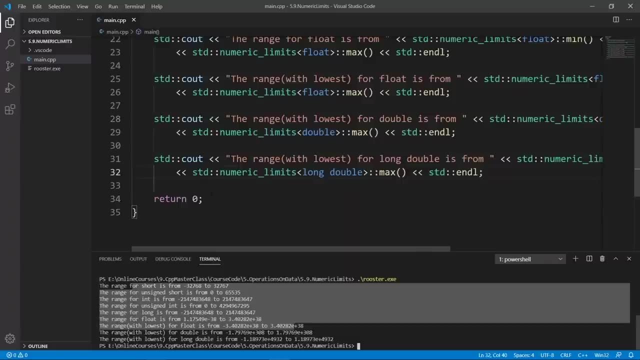 a much easier way here. This is an option you can use, or you can even use the integrated terminal inside Visual Studio Code here, like we've been doing all along. There are a few other facilities you can use in this library of limits. For example, we can try and print out if a number is signed, or 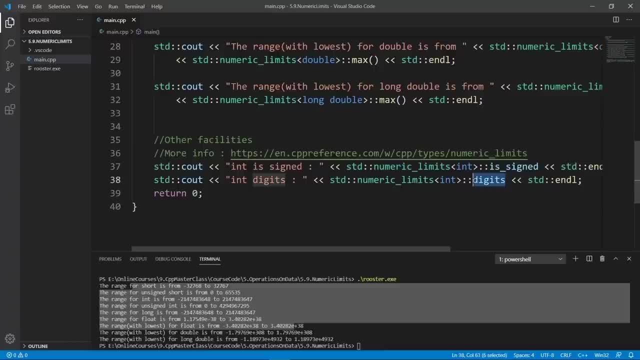 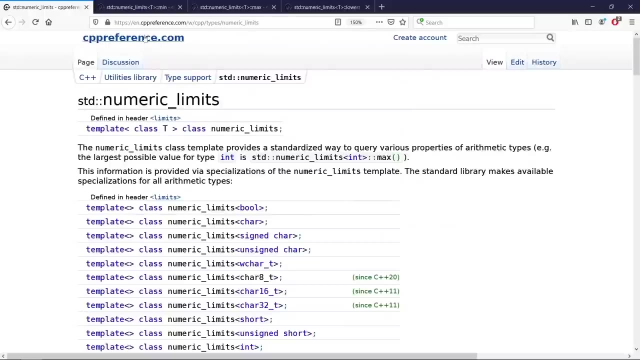 unsigned, or get the number of digits we can represent in an integer type. These are a few examples. I just chose because they are easy to understand and really helpful, but you can find more about this later. This library in the documentation, and if you come here at cppreferencecom- the link is here. 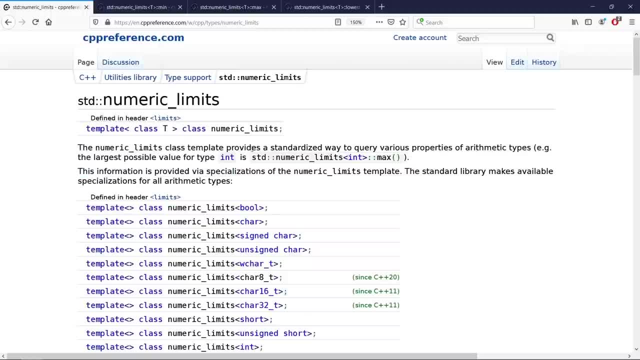 you can really find all about this library here. This library provides a standardized way to carry various properties of arithmetic types. For example, the largest possible value of type int is this, and we have a bunch of things we can do here. Don't be scared off by this template thing. 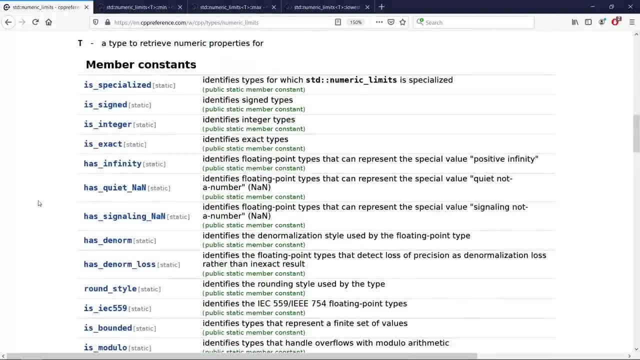 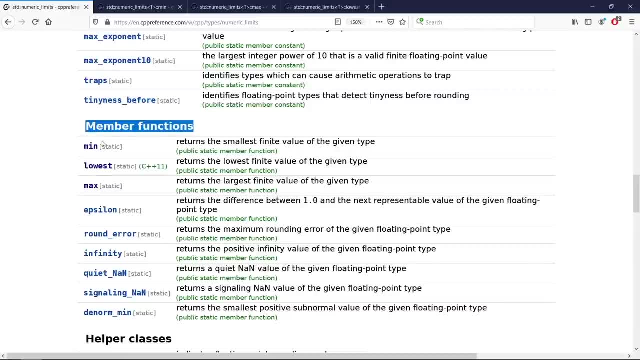 Just think of them as placeholders For the type for which you are trying to query information, for There are a few functions you can call on these things. For example, there is mean lowest max that we just played with in Visual Studio Code, but you can see that there are a lot of things you can play with, especially if 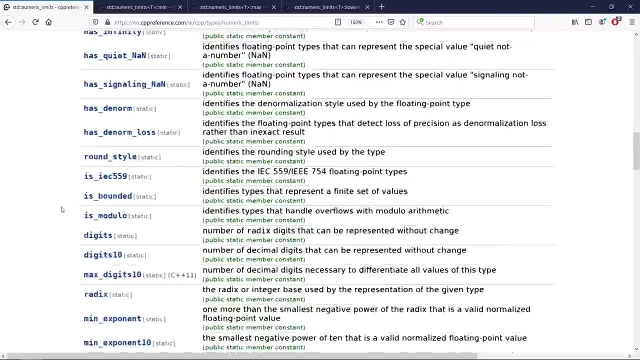 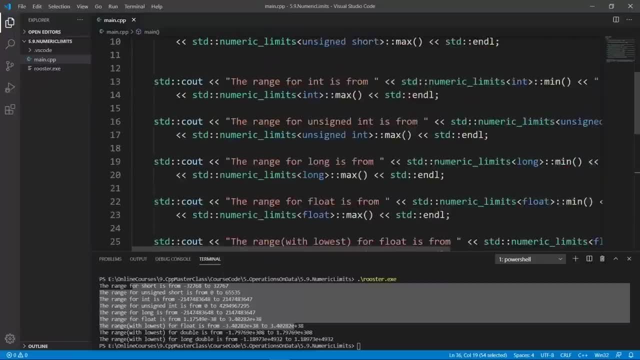 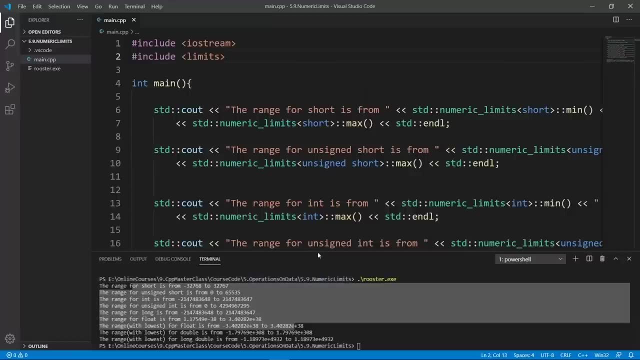 you have some math background to understand all these concepts here. You can play with this and see if it is helpful for whatever application you are doing. Okay, this is really all we set out to do In this lecture: to learn a little bit about the limits library. it is helpful in trying to 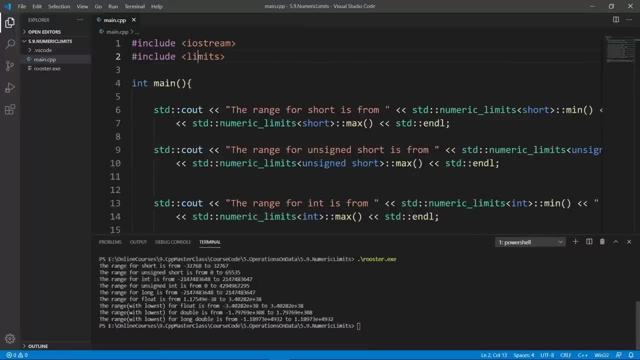 understand the ranges for your types. If you happen to need these kinds of things, this is going to come in handy. We're going to stop here in this lecture. In the next one we're going to learn about some math functions we can use in C++. Go ahead and finish up here and meet me there. 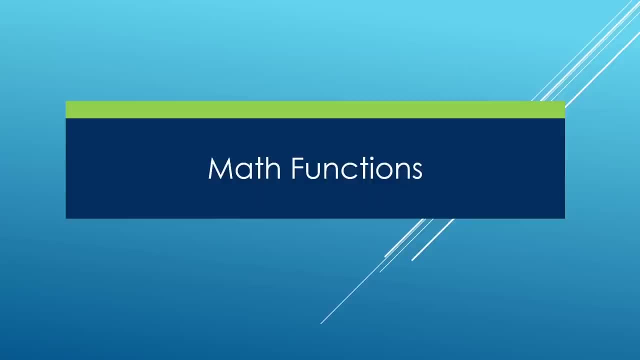 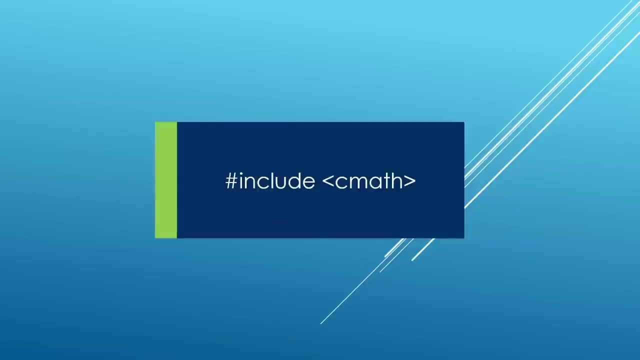 In this lecture we're going to learn about math functions, and these are functions that are built into the C++ library- C++ standard library- that we can use to do some math. If you are doing some math operations, you're going to find this helpful. They live in the C math library and if you want to use them, you're. 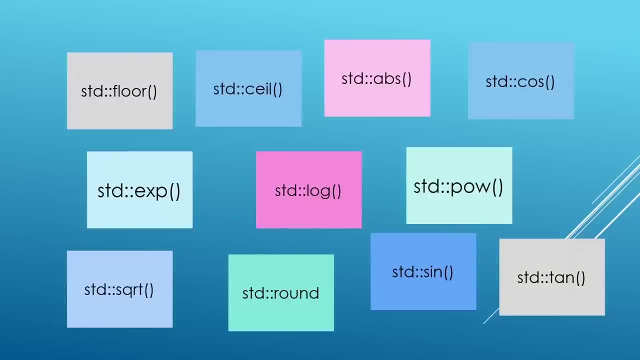 just going to include that and you're going to have access to them. What you see here is a simple summary of some of the things you can use in these math functions. You can use std floor to round down or std seal to round up. 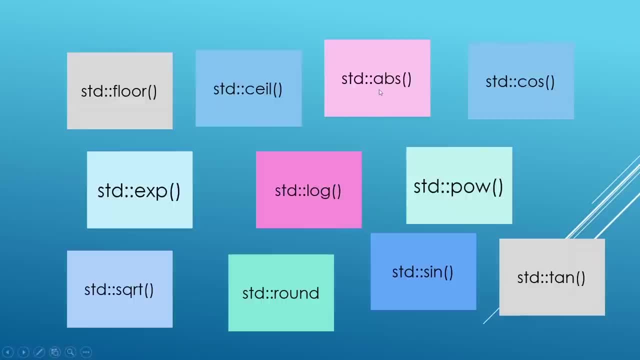 You can use the abs function to compute the absolute value of a number. You can do trigonometry, You can do the cosine sine and things like that. You can compute the exponential of a number. You're going to see what this means in a few lectures. You can use std log and again, if you 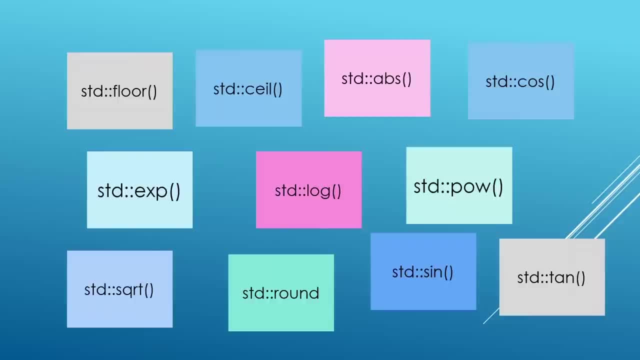 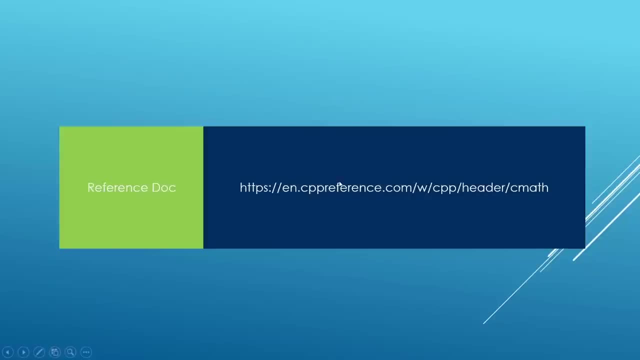 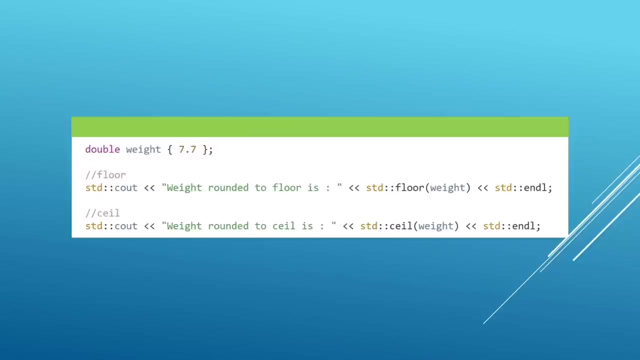 have some math background, these concepts are not going to be foreign to you. Many of these functions are documented here at CPP Reference, so it might be worthwhile to go there and check them out. Here is an example of something you might want to do. For example, you have a variable. It's called 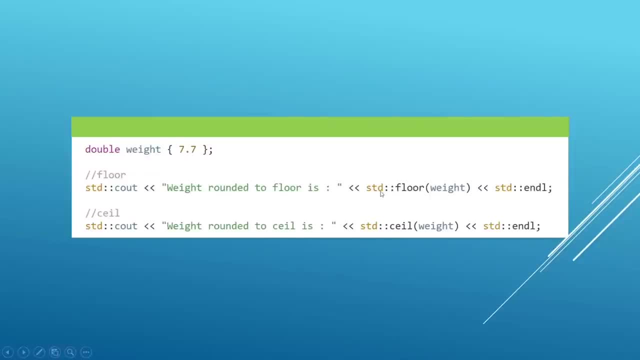 weight Inside we have a 7.7, and if you do std floor of this variable, this is going to be rounded down to a 7.. If you want to round up, you're going to use std seal and you're going to get that. 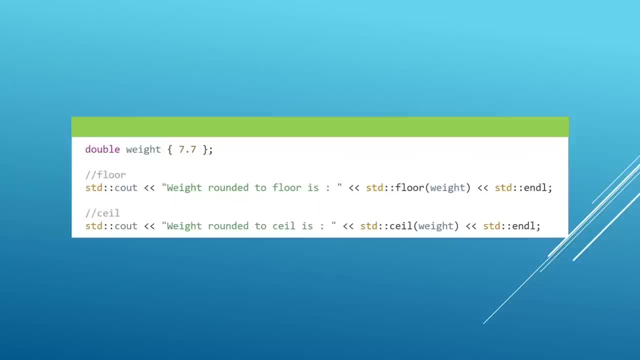 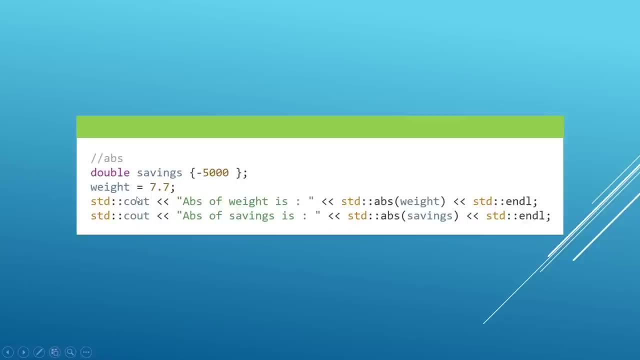 and we're going to see what this is going to give us in a minute. when we hit Visual Studio Code, Here is how you would use the absolute value. You have a few variables here, and if you try to plug them in this absolute value function, 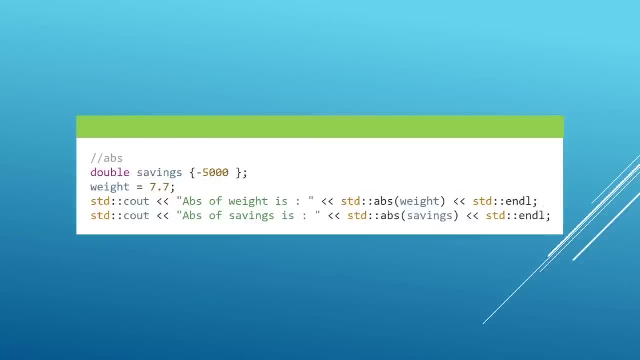 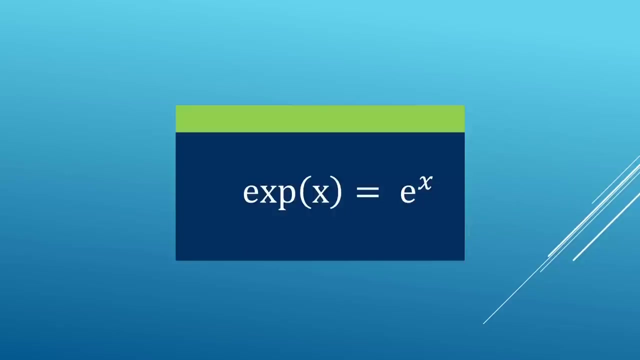 you're basically going to get the weight of the number, without any sign in front of the number. positive or negative, The absolute value is the weight of the number, without caring about the sign, if I may say it like that. Okay, we also have the exp function which is going to compute. 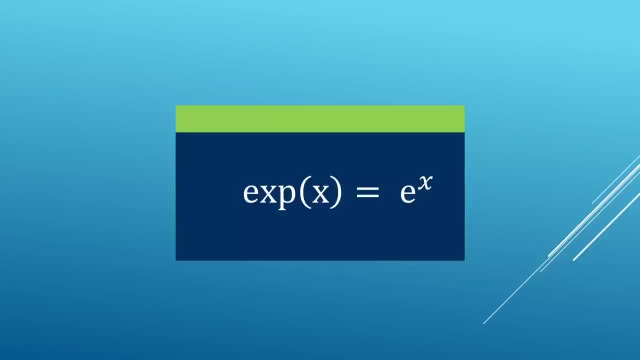 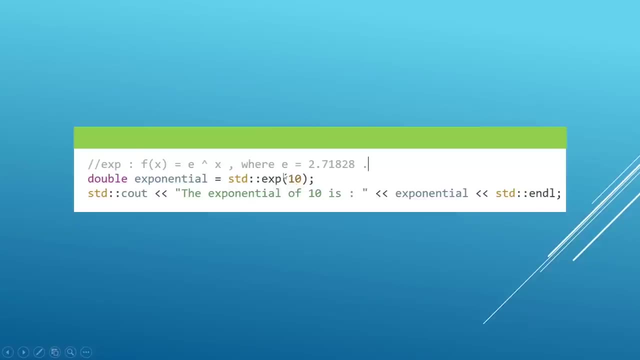 the exponential of a number. This is a math concept, so if you don't have the exponential, you don't have a background in math. This is going to be a little hard to wrap your brains around, but in math we have this number which is called e, and its value is approximately 2.71828,. 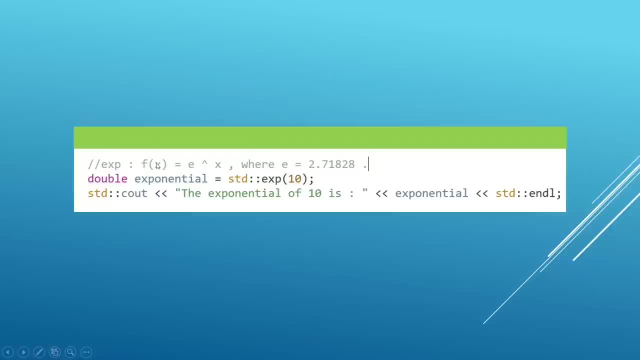 like you see, here The exponential function is going to do what fx here is doing. It's going to take e and elevate that to the power of x and for example, in our code here we're going to get the exponential of 10, which is going to be e. 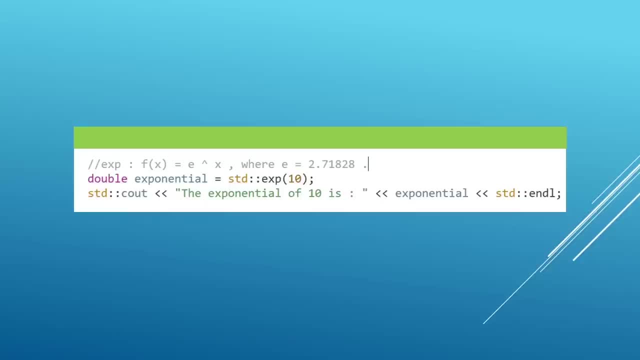 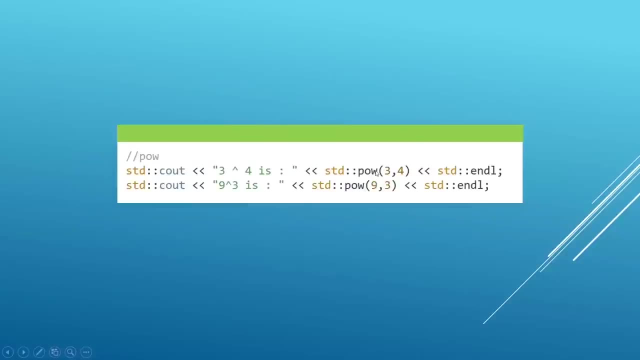 And we're going to play with this in Visual Studio Code and you're going to see the value of this. We also have the power function here, which is going to take the first parameter and elevate that to the power of the second parameter. So this is going to be 3 to the power of 4 and 9. 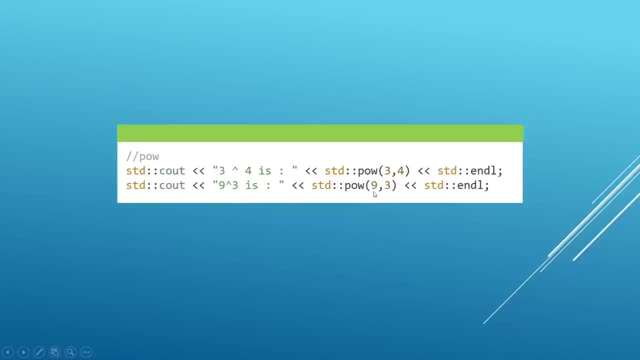 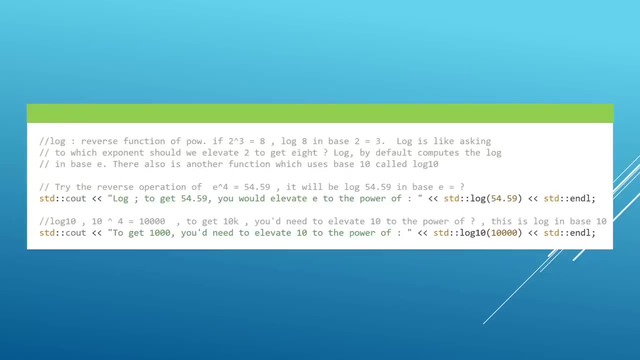 to the power of 3, and we're going to get the answer if we plug this into Visual Studio Code And we have log functions, which is basically the reverse of the power function that we just looked at. If you do log 8 in base 2,, for example, 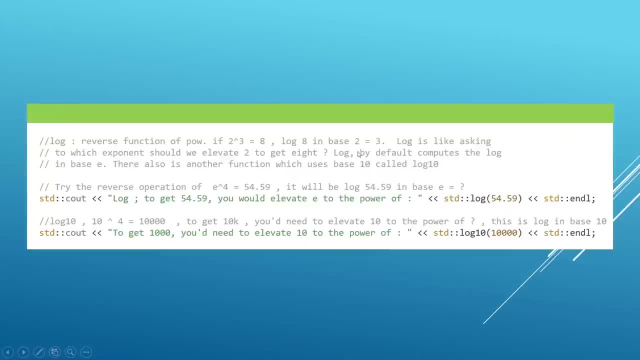 it is like you are asking: to which power should I elevate 2 so that I get 8?? And the answer here is going to be a 3, of course, But the catch is that the log function by default works in base e. So what we are asking, for example, if we say log 54.59, is: 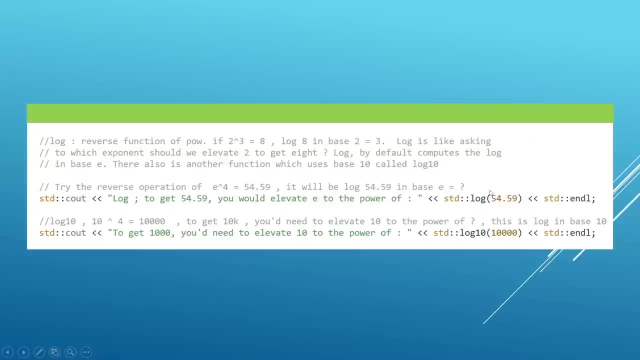 which power should we elevate e to get this number in here? And it is going to be computed and you're going to see this if you plug this into Visual Studio Code or you can try to use one of the calculators available to you, and you're going to see that this makes sense. 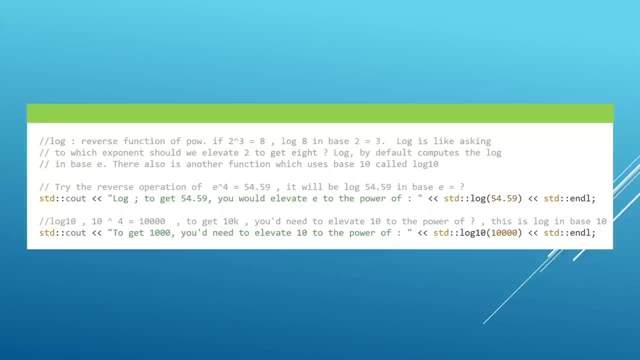 We also have a special function that is going to do the same thing, but in base 10, and this is going to be easier to understand. For example, here we are computing log 10.. What we are really saying is: to which power should we elevate 10 to get 10,000?? And this is. 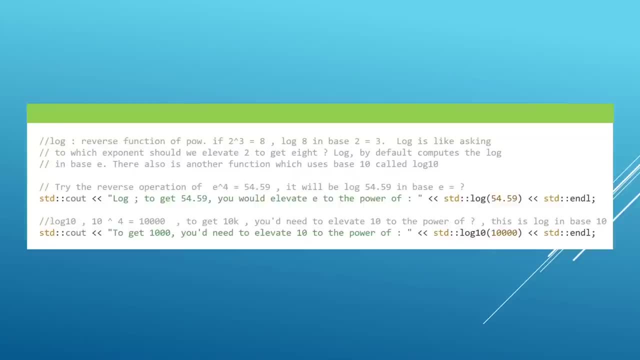 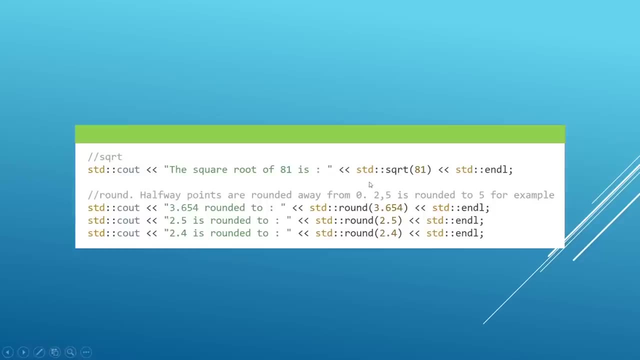 easy, because the answer is a 4.. 10 to the power of 4 is 10,000.. I really hope this makes sense. We also have a square route function we can use, So square route of 81 is going to be 9.. 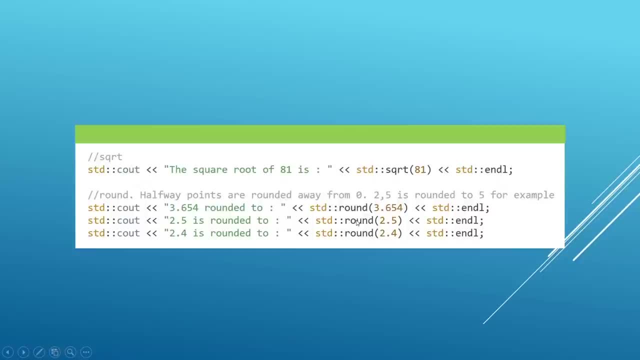 We have a function called std round, which can round, And what it's going to do. by default, half of the log function is going to be 9.. So we're going to have a function called std round. points are going to be rounded away from 0. So if you have a 2.5, it's going to be rounded up to a. 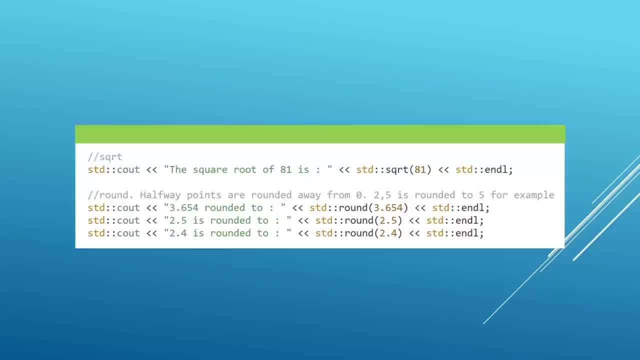 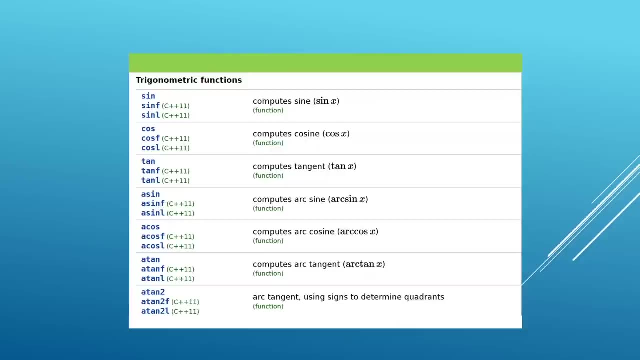 3. And if you have 2.4, it's going to be rounded down to a 2.. We also have a host of functions we can use in trigonometry. We have a sine function, we have a cosine function, we have a tan function. 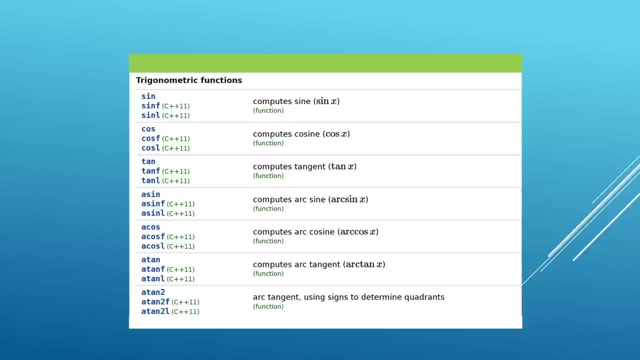 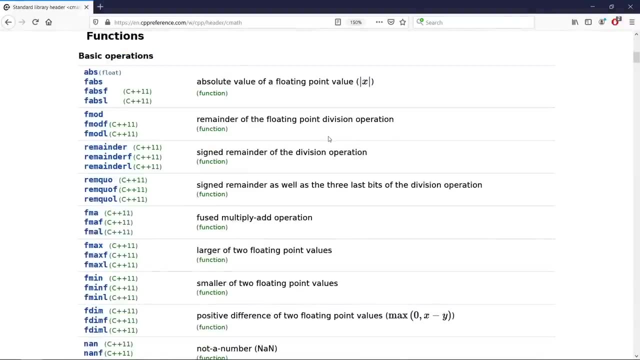 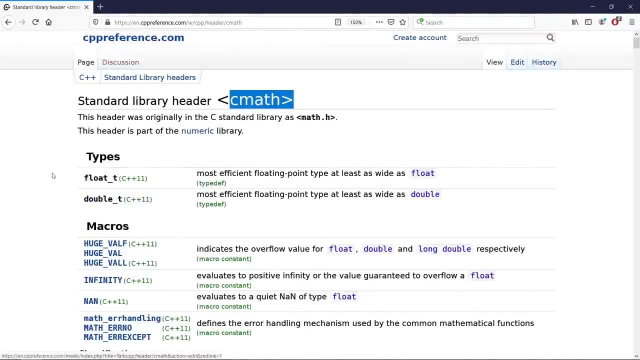 If you know these concepts in math, this is going to come in really handy if you want to do this. I have to say that what we just talked about is the small set of what we can do with these functions here in CMath And we are here at cppreferencecom. 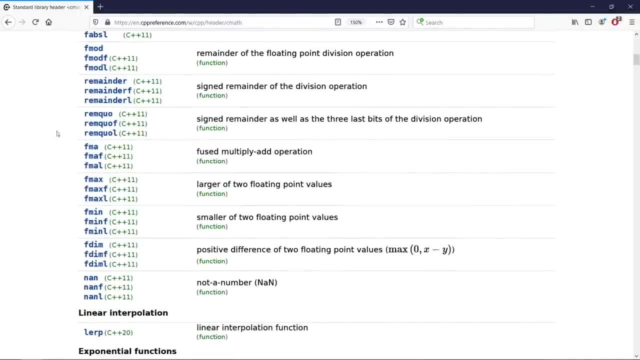 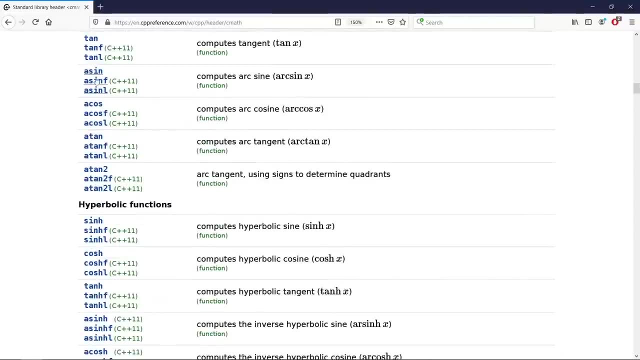 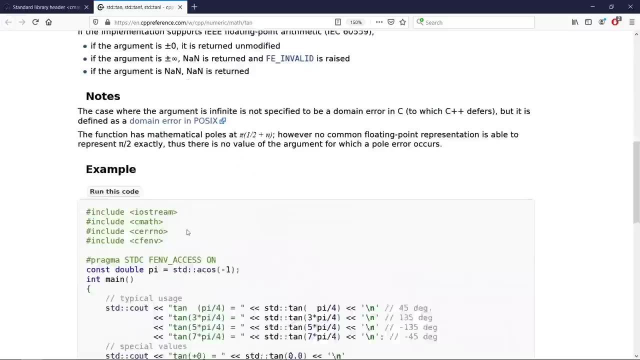 and we can see all these functions here. We can do reminder, we can do fmin And, if you want, you can check these out in the documentation. For example, if you go to tan here and click on it, you are going to get the description and explanation of what this function does. 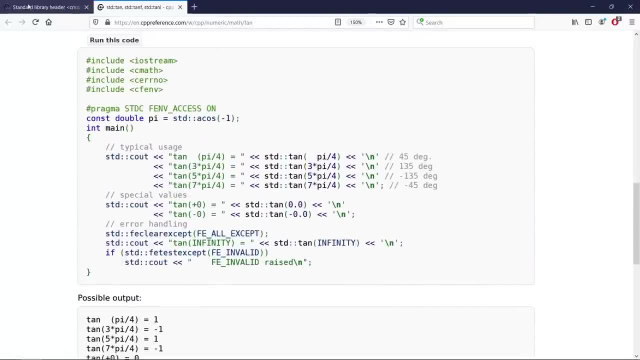 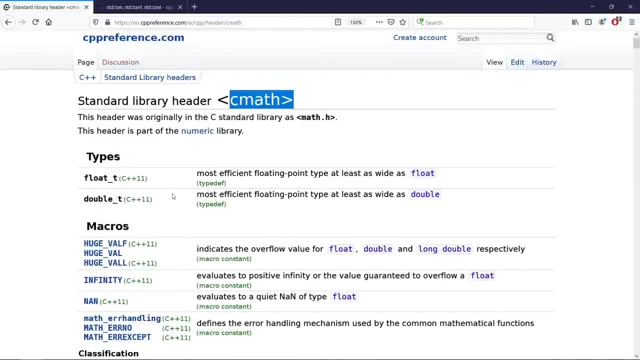 And you're going to have a simple example of how you can play with us. Okay, now I hope you have a better idea of what we can do with these functions in the CMath library. We're going to head to Visual Studio code and play with some of. 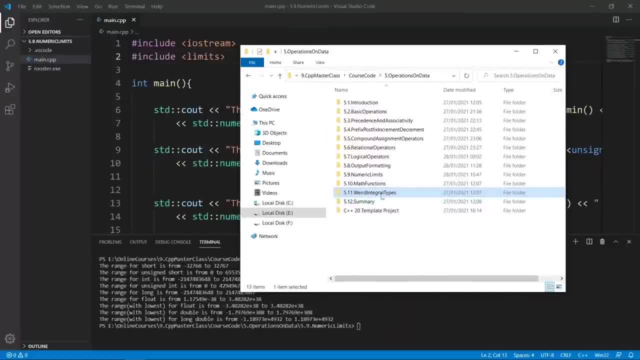 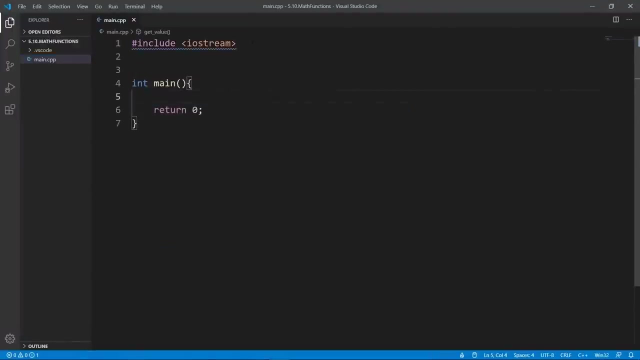 these functions. Here we are in Visual Studio code. The current project we're going to work on is math functions. We're going to copy over our template files And we're going to put them in our directory here: math functions. Open this up in Visual Studio code And we are going to remove whatever it is we don't need And we are going to. 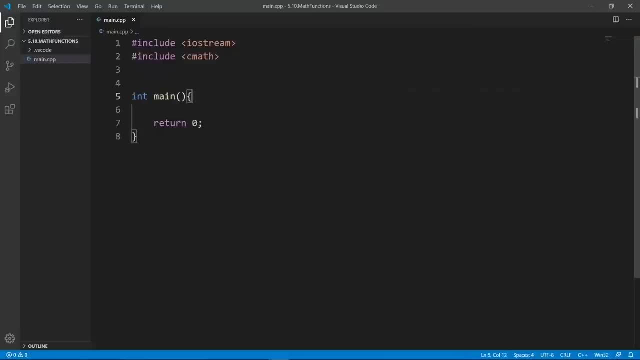 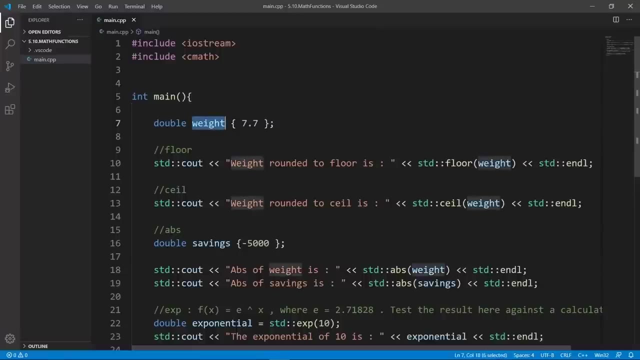 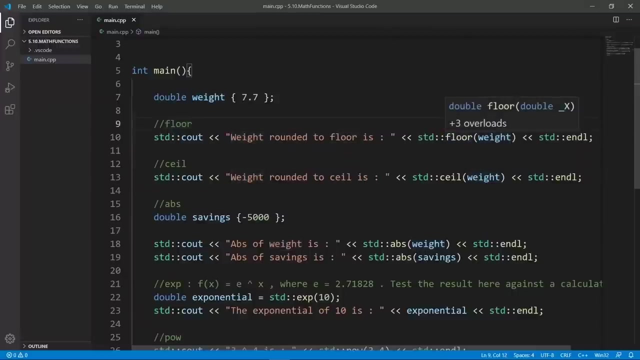 include our library, which is CMath, And we are going to put in our code so that we can play with us. And here we have a variable called weight And we're going to try and use a few math functions on it So we can use std floor to round down. 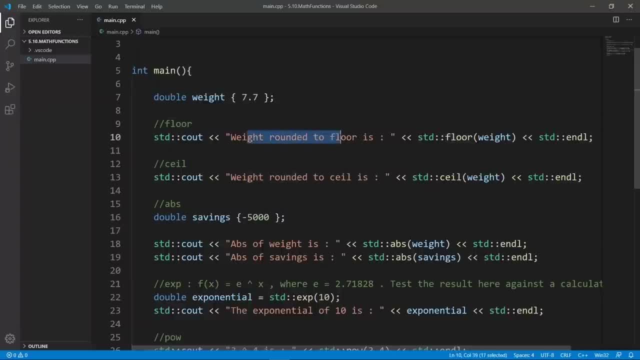 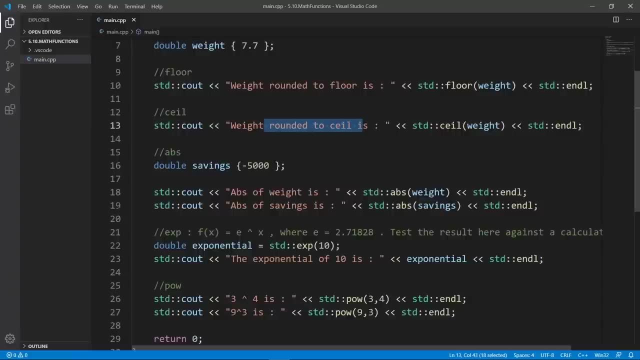 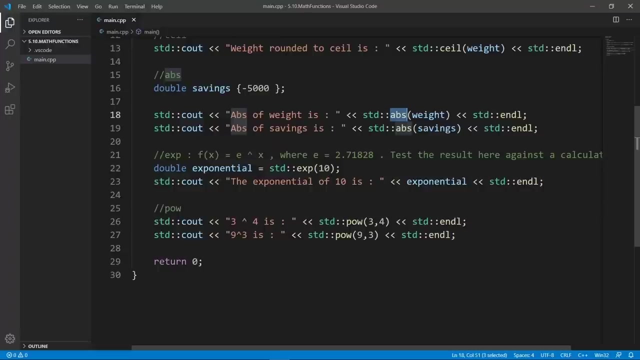 and std sale. to round up: So, weighted, rounded to floor is going to be printed out And weighted, rounded to sale is going to be printed out. We're going to have a number here In this savings variable. it's going to be a negative number And we're going to try and compute the absolute value of this. We're going to see it printed out. Another thing we're going to compute is the exponential of the value. We're going to do std exp 10. And what this is going to do is going to take e and 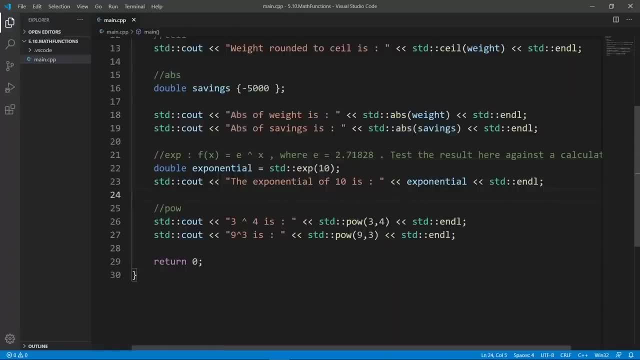 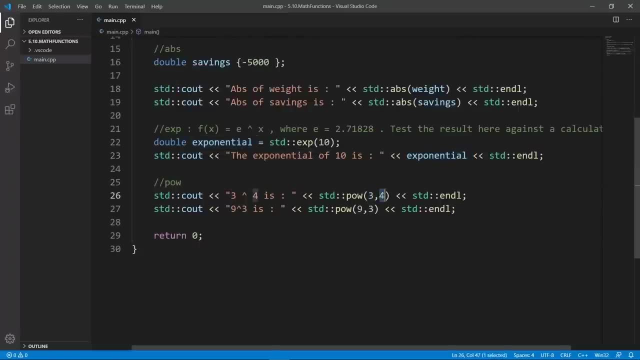 raise it to the power of 10.. And that's what we're going to get printed new. The other thing we want to do here is compute the power of a number. We're going to take three and raise it to the power of four, and 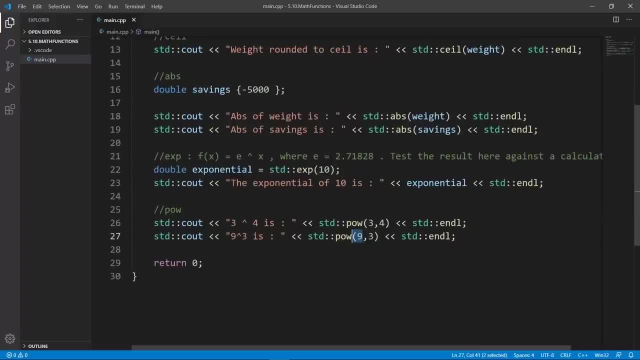 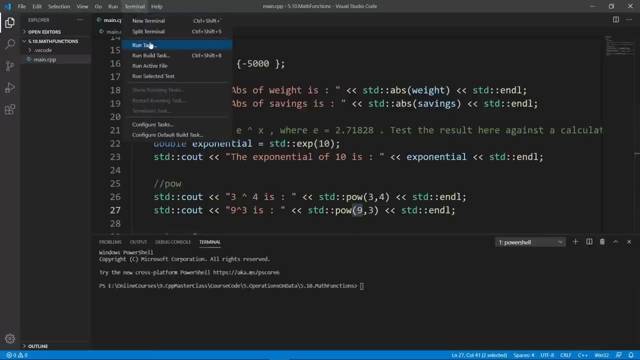 take nine and raise it to the power of three and we're going to see what these things evaluate to. we're going to open up our terminal here and we're going to run the tests to world with GCC. the world is going to be good And if we run roaster, we're going to get to these. 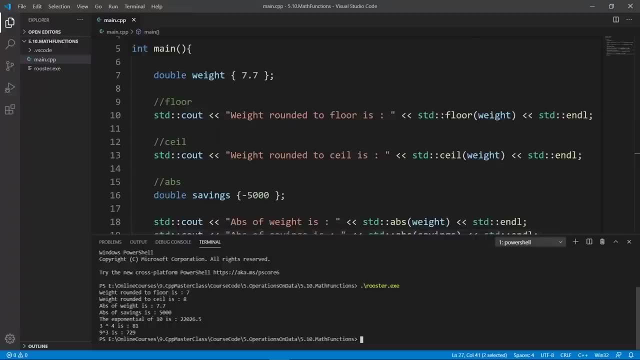 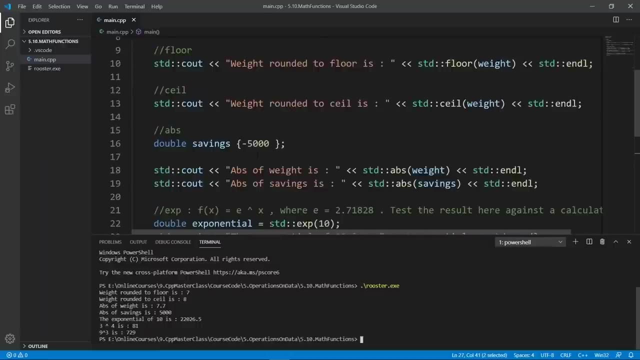 things here. so 7.7 rounded to floor is going to be 7. so we're going to round down: 7.7 rounded to seal is going to be 8 and that's what we're going to get and the absolute value of weight is going. 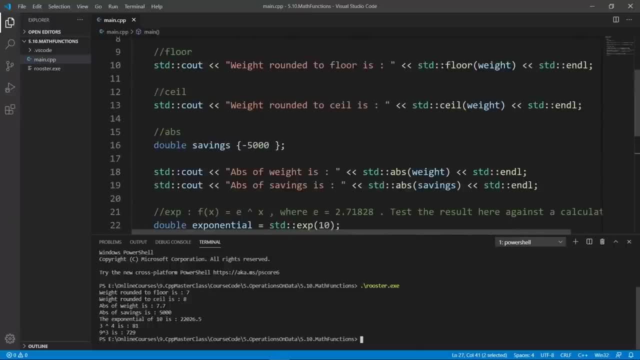 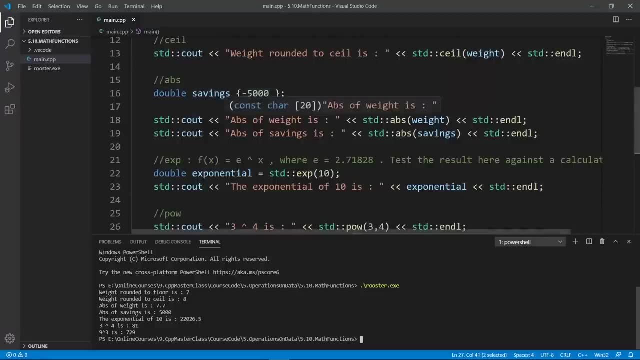 to be 7.7, because it is a positive number and the absolute value of minus 5000 is going to be 5000. and again, when you compute the absolute value of something, you are interested in the weight of that thing, without considering the sign, without really worrying if it is positive or negative, you just 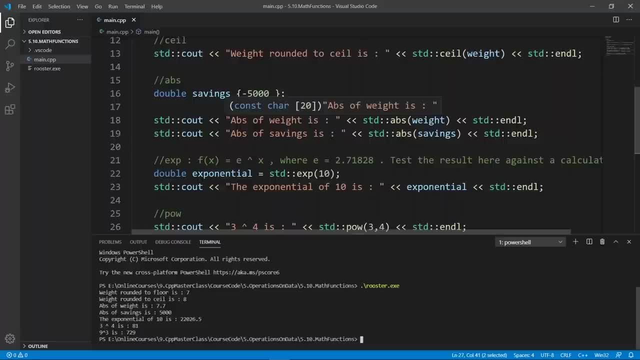 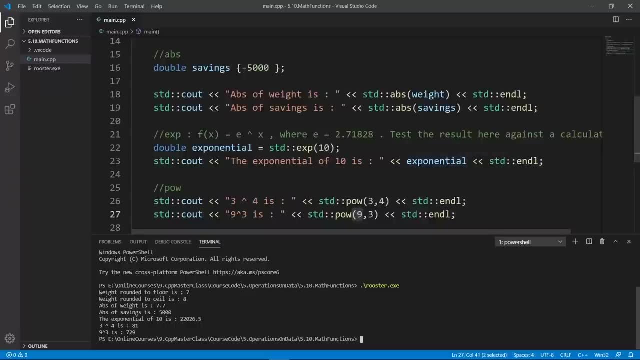 want to get the magnitude of a number. that's what we use in math to mean that magnitude. okay, so if we go down, we're going to get the exponential of 10 is exponential and you're going to get that here and again, what this function does. 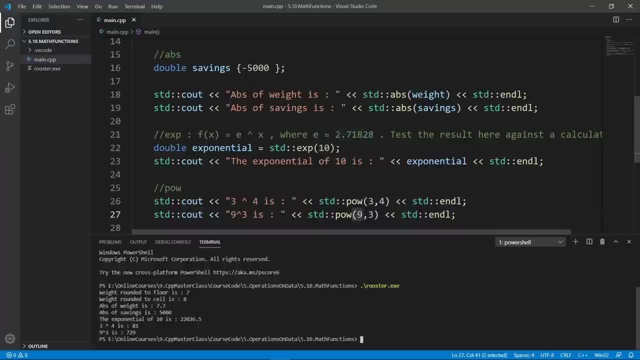 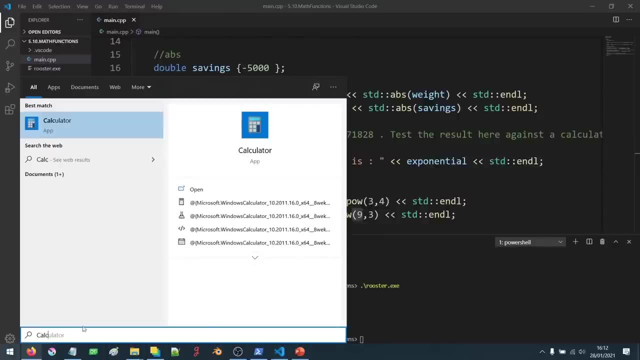 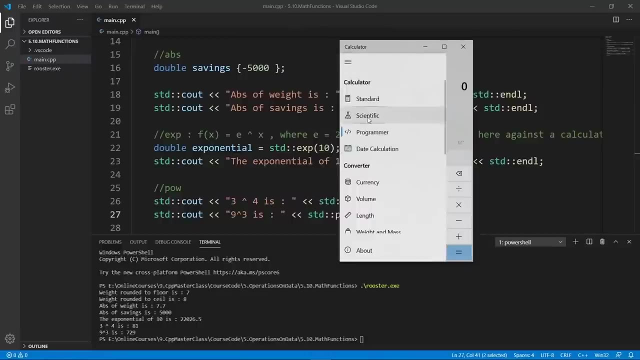 is: take e and raise it to the power of 10, and that's the answer here. we can try and prove this with a calculator. so i am going to open my windows calculator. you can use whatever calculator you have access to. i am going to use a scientific calculator here and you see that we can hit e. 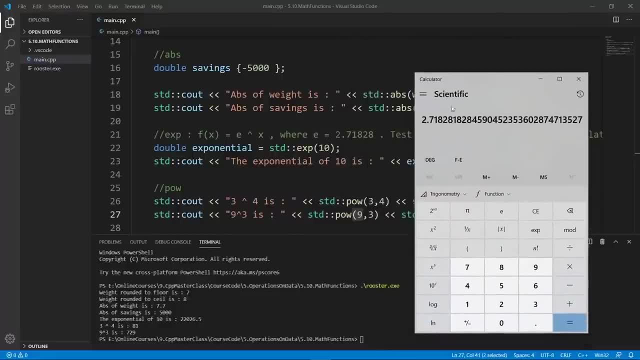 and we're going to get the value of this e number in math. here it is simplified. but if i take it and raise it to the power of 10, the answer is going to be 22.026. and if we look in our program we have: 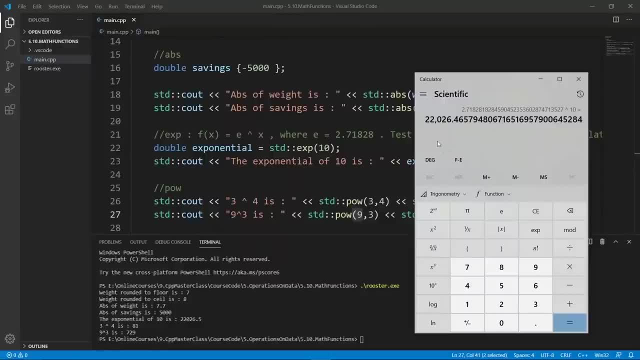 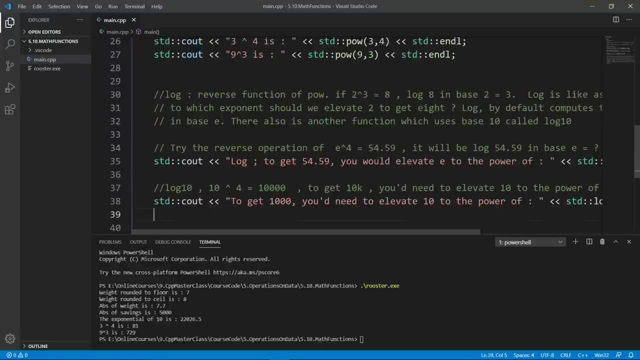 22.026.5. okay, it is rounded up a little bit, but it is almost the same thing. okay, we also want to play with log functions a little bit. log is basically the reverse of the power function and we just talked about this in the slides. but if we do log 8 in base 2, we are basically asking: to which power should we raise? 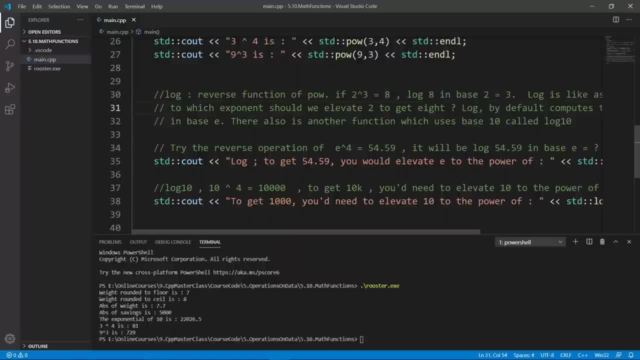 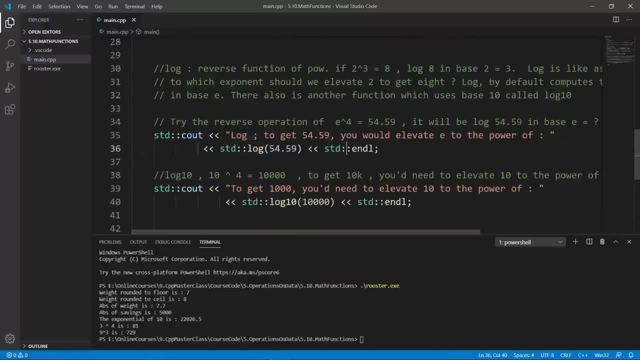 2 to get an 8, and the answer to that is going to be what this log number in base number is going to evaluate to. the catch is that the log function, if you use it row like this, it is going to be using base e, and we just saw that e is 2 to the power of 7 or something. let's go back to our 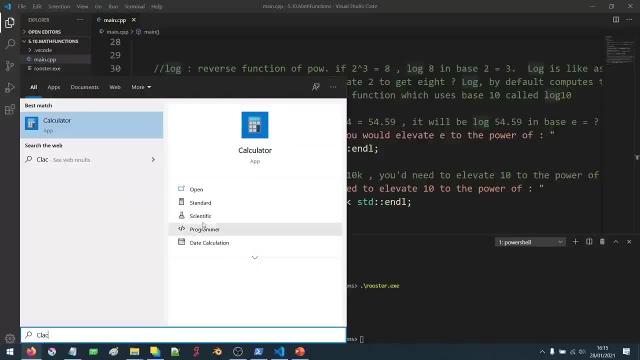 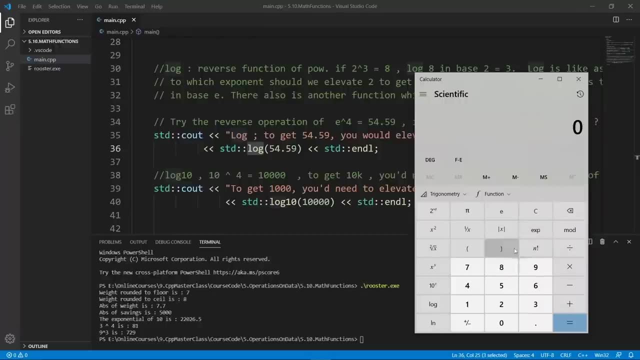 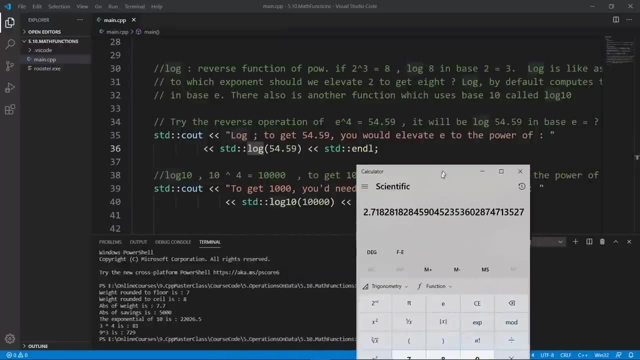 calculator and see if we can see that. why not? why try to guess when we have a good calculator in our hands? we are using the scientific calculator. so if we hit e here, this is the value of e. okay, so when we do log, we are basically asking: to which power should we raise e so that we can get? 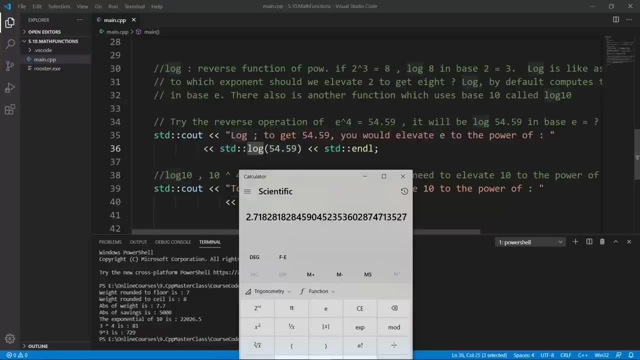 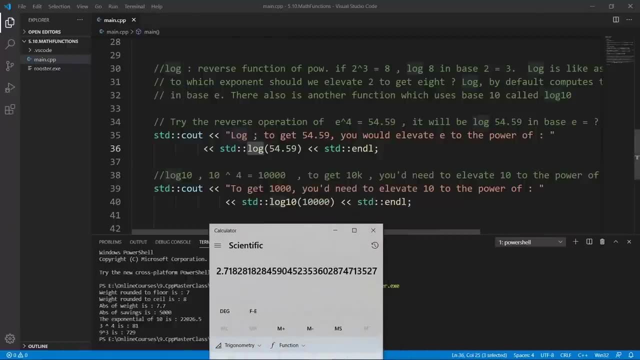 this 54.59 and the answer is going to be computed and printed out here. we have a version of the log. this that is going to use base 10. so if we use this, we are basically saying: to which power should we raise 10 to get 10 000? and the answer is going to be printed out here and it is going to be a 4. 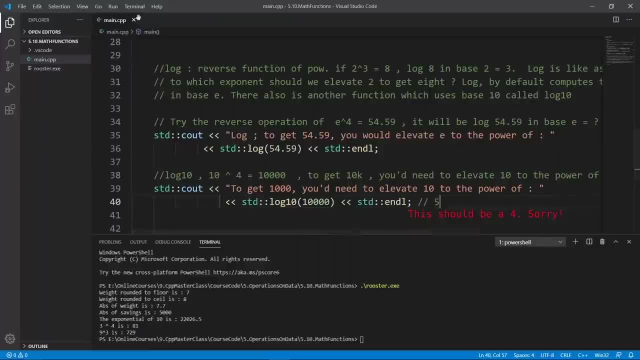 because this is easy to do in your mind. so let's run this. we're going to world the task. we are going to run the task to world with gcc and we're going to run our program and we're going to get our output here to get 54.59 and we're going to run our program and we're going to run our program. 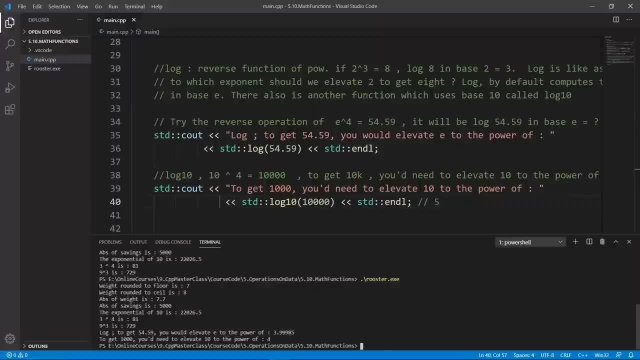 dot 59, you would elevate e to the power of this number. here this is the answer and, if you want, you can prove this with your favorite calculator. you're going to get something close to this. to get 10 000, you'd need to elevate 10 to the power of 4. that's what we're going to get in here. let's 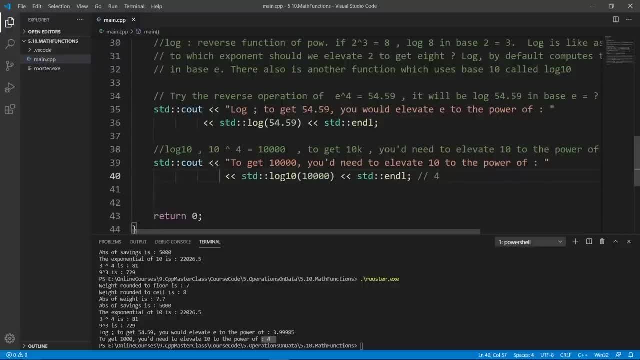 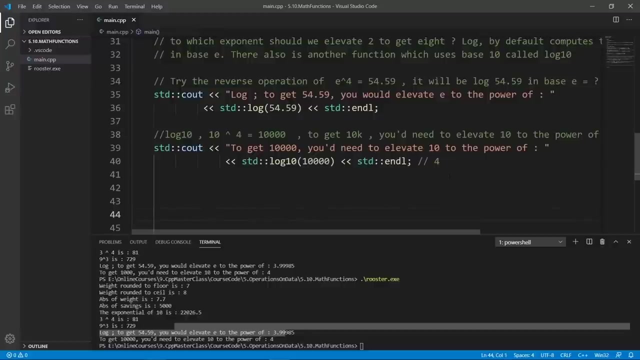 print this out again. many mistakes, sorry, but i hope you get the point. if we build again so that we can see things properly and run, we're going to get proper data and this is really what we expected to get. we have a few more functions we can play with, as we saw in our slides. let's play. 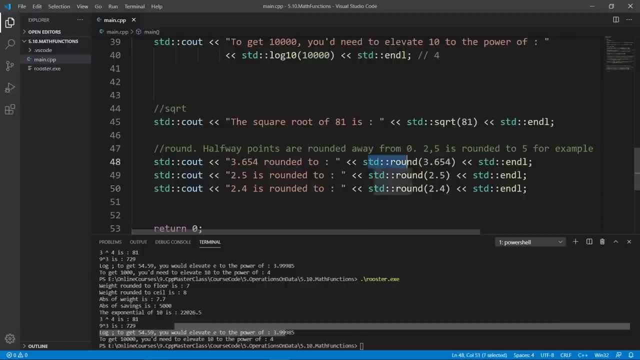 with square root and the std round function. here we are going to get the square root of 81, we're going to get it printed out and we're going to see what std round does. it is going to round away from zero if we are at half point. 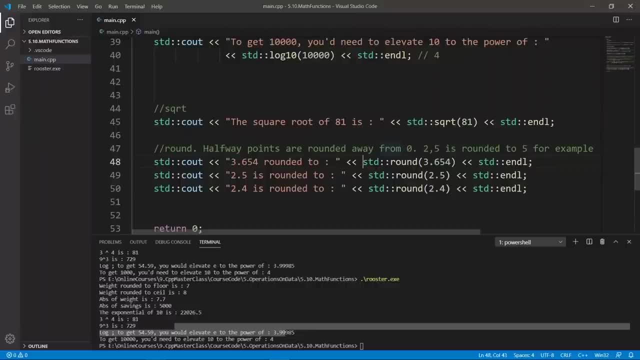 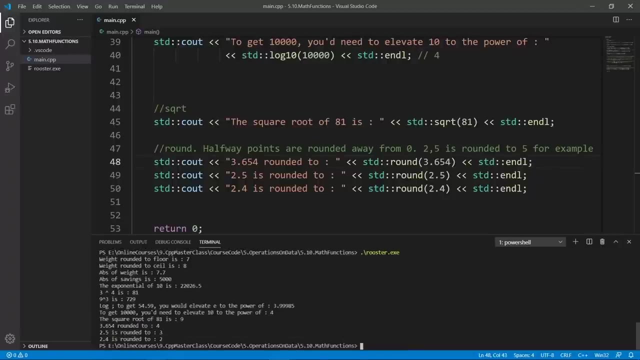 and if we are not at half point, if we are below that, we're going to round down. if we are higher than that, we're going to round up. we're going to run this so that you can see this running and we're going to call rooster and the 2.5 is rounded to 3. 2.4 is rounded to 2. 3.6 is rounded. 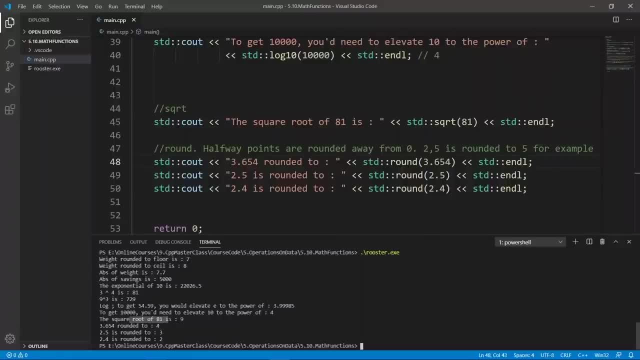 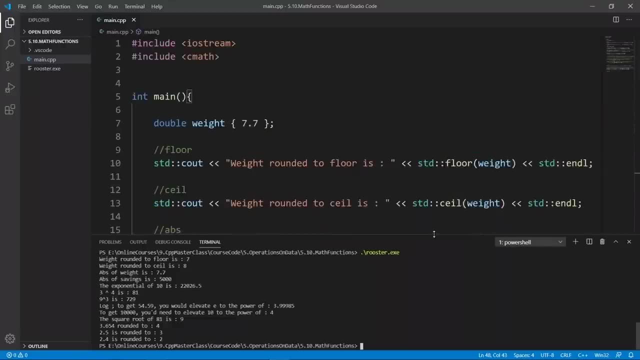 to 4. this is what we expect, and the square root of 81 is 9. this is really all we set out to do in this lecture. to play with a few of these cmath function. they are not really hard to use once you have the basics of math nailed. 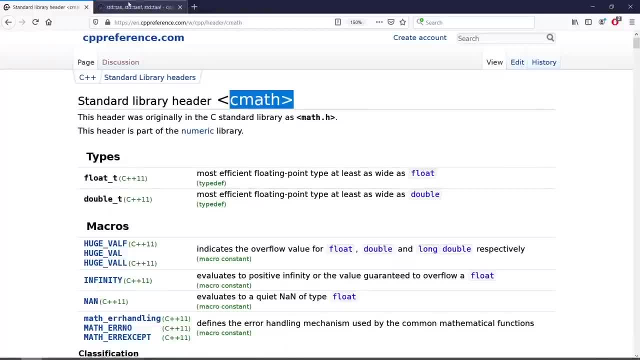 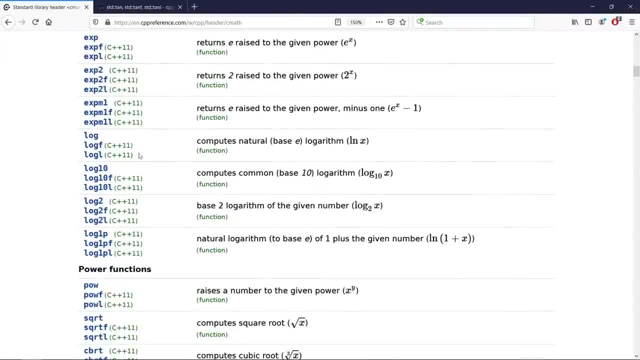 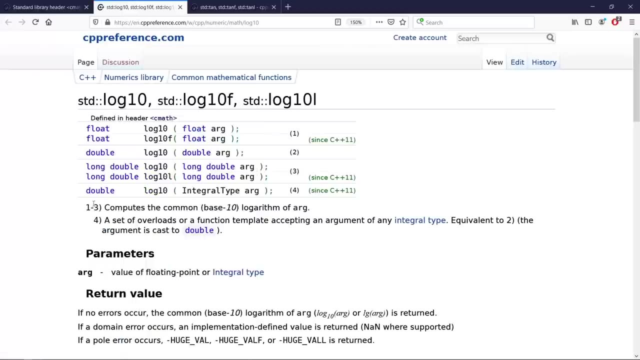 down. and again, if you want to check the full list of these functions, please come to our reference documentation. here you're going to find a lot of them. and if you want to see how to use one of these, for example, if you click on log 10, here you're going to come, here you're going to get. 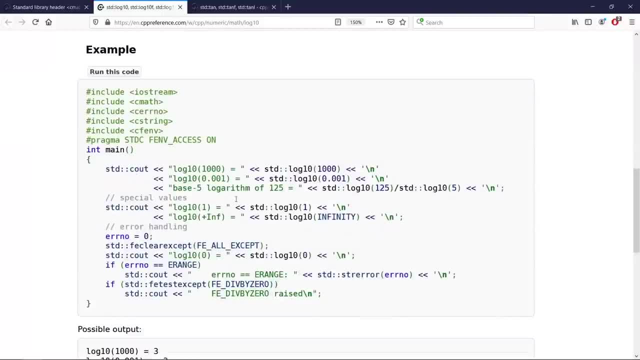 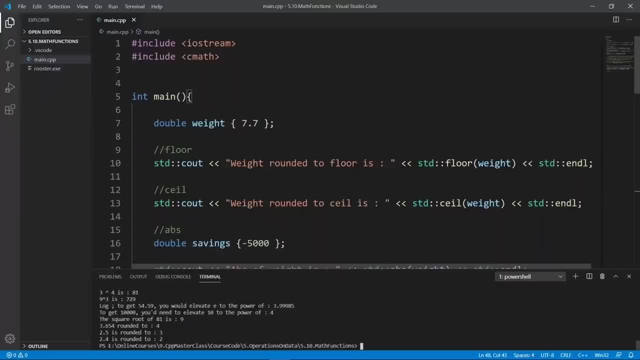 an explanation of the function. and, even better, you're going to go down and get a nice piece of math and play with and really make sense of what is happening in these functions here. this is really all we set out to do in this lecture. I hope you found it interesting. we are going to stop here. 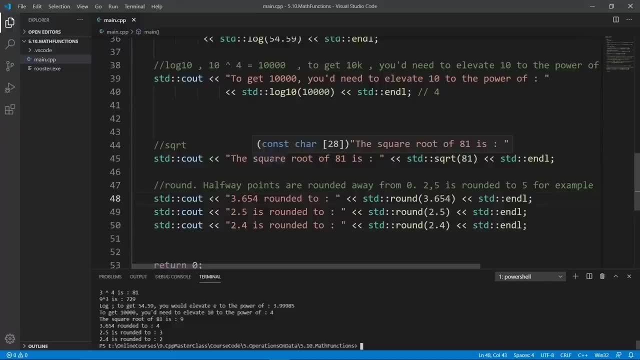 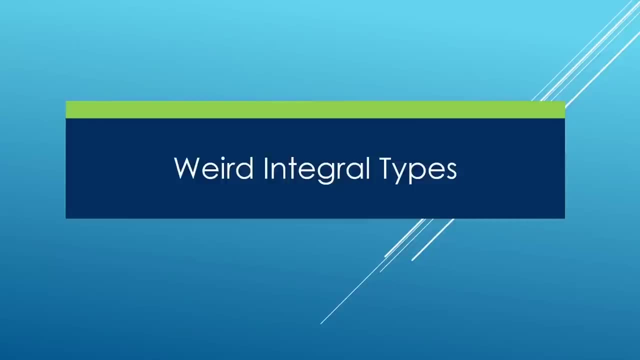 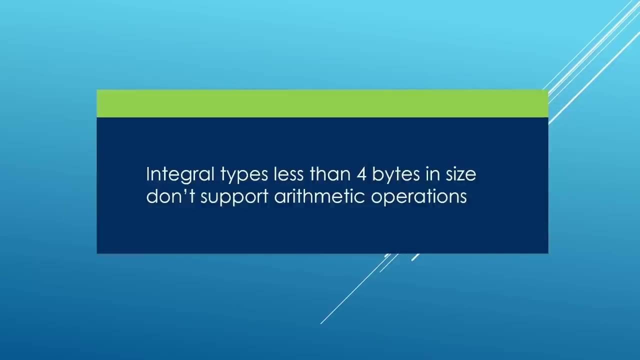 in this lecture. in the next one, we're going to learn about some weird integral types. go ahead and finish up here and meet me there. in this lecture, we're going to learn about some weird integral types, and what do I mean by this? well, if you look here, integral types less than four. 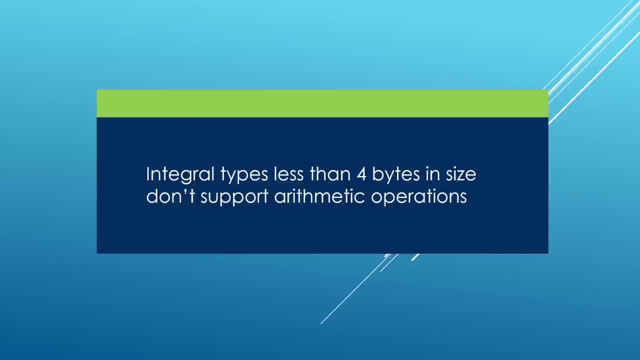 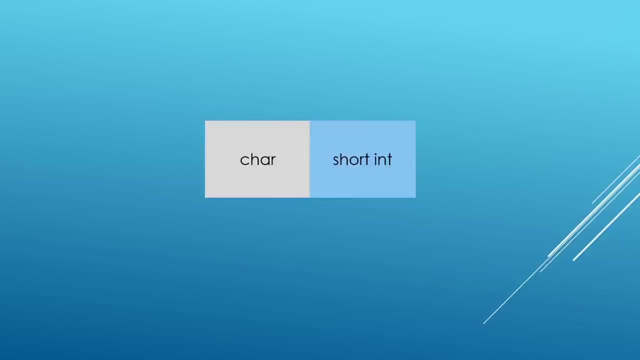 bytes in size don't support arithmetic operations and these are operations like addition, subtraction, multiplication, division. you can't do these operations on those types, and here I have an example of some of those types. we have a car: it is one byte in size and short ant is two bytes in size on most processors. 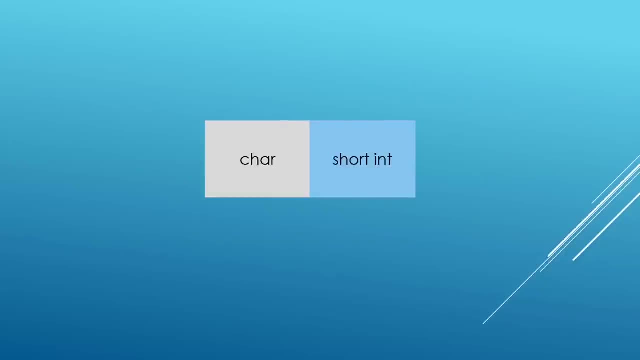 so you can't do arithmetic operations if your integer value is stored in these times. well, this has to do with processor design and they decided to choose ant as the smallest type- integral type- for which they can do this arithmetic operations. but compilers are really smart enough to notice if you are trying to do arithmetic operations on these types and they are going. 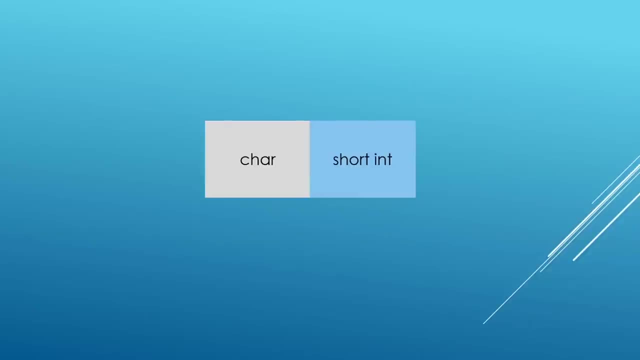 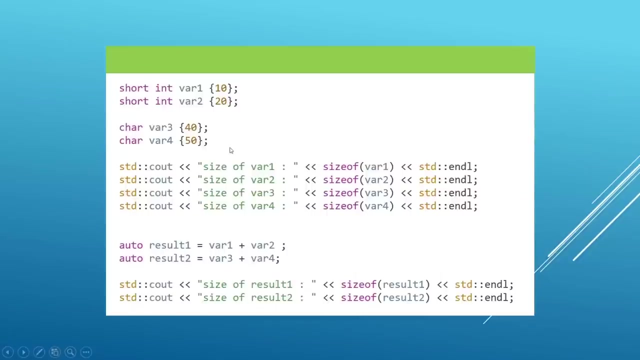 to implicitly convert from these smaller types to ant, and this is something you need to be aware of. if we look at this program here, for example, we have var1 and var2. they are stored in variables that are of type short ant, and we have var3, var4, which are stored in a variable of type car. we can try and print their sizes and 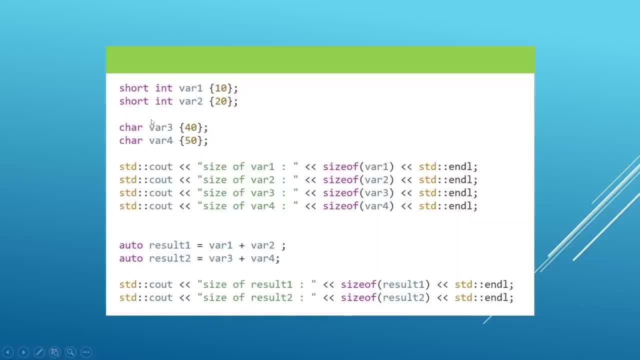 we're going to get two, two, one one for these variables, because a short ant occupies two bytes in memory for my computer here and the car occupies one byte in memory. but the catch is that the result is the same type as the things you added up down here. if you try to add them up. 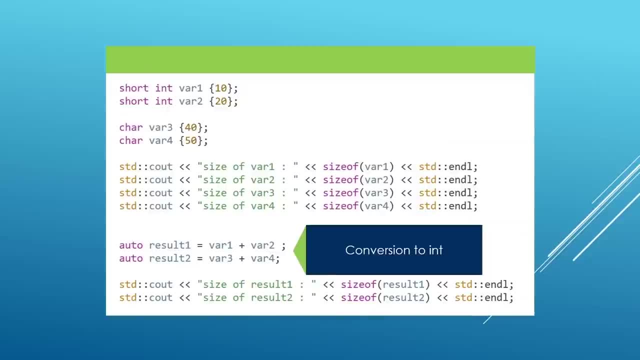 the result is not going to be the same type as the things you added up and you would expect auto to deduce to the same type as var1 and var2, and it's not. result is going to be an integer, because ant is the smallest type for which we can support these arithmetic operations. so if we print, 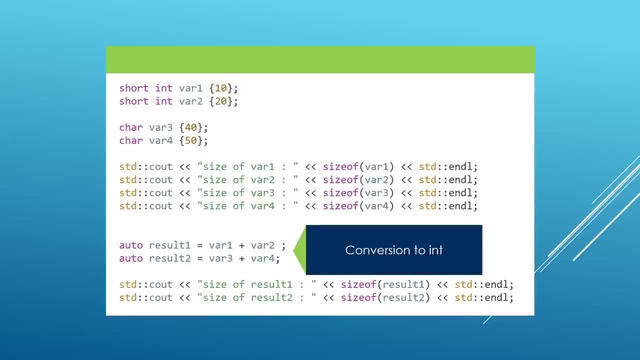 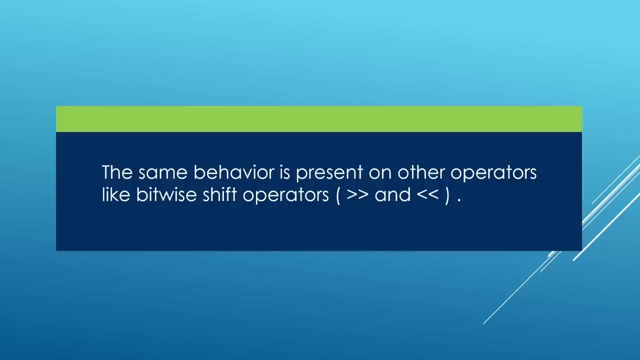 the size of result one and research two. we're going to get four, but this is the behavior in you're going to get and we need to be aware of it. the same behavior can be observed on other operators that we will have a chance to look at in a few chapters ahead, and these are called shift. 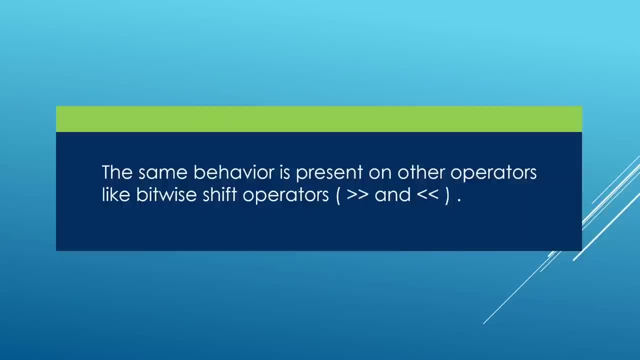 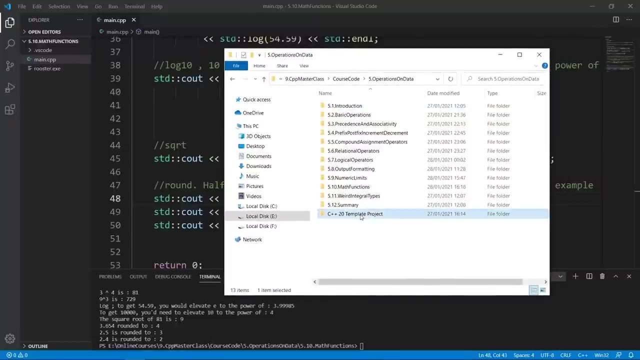 operators. you use them to shift bits, but i don't want to talk any more about them because we're going to have a chance to learn about them in detail. okay, now it's time to head to visual studio code and actually see this in action. here we are in our working directory. we are going to 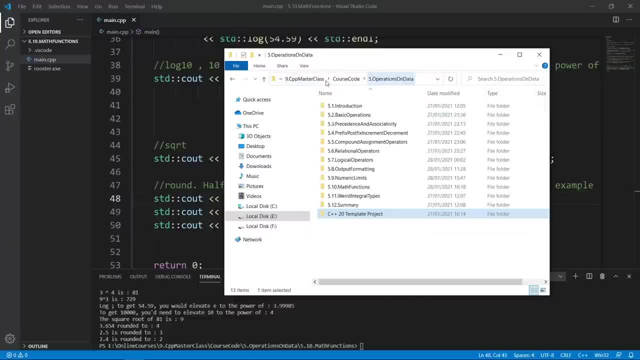 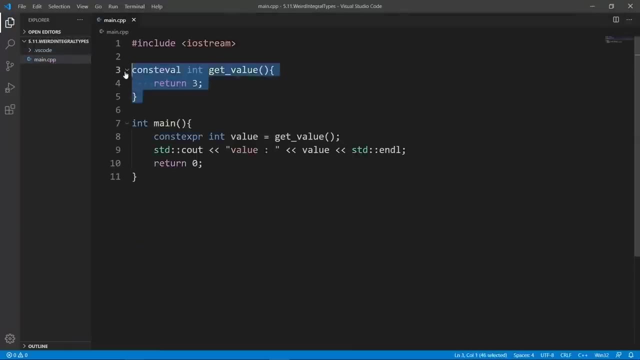 copy our template project. we're going to copy this quickly. put that in our folder on weird integral types. this is our current project here and we're going to open this up in visual studio code. we're going to open this up and we're going to open our main cpp file. remove whatever it is. 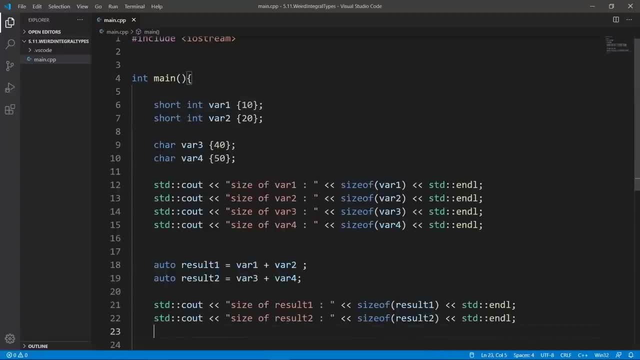 we don't need and we are going to put in our code. this must be very familiar, because it is what we just saw in the slides. so what we are doing here we have four variables. var1 and var2 are short, and so these are going to take two bytes in memory on my computer here. 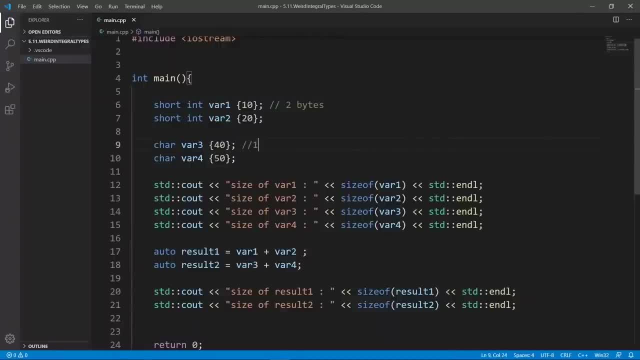 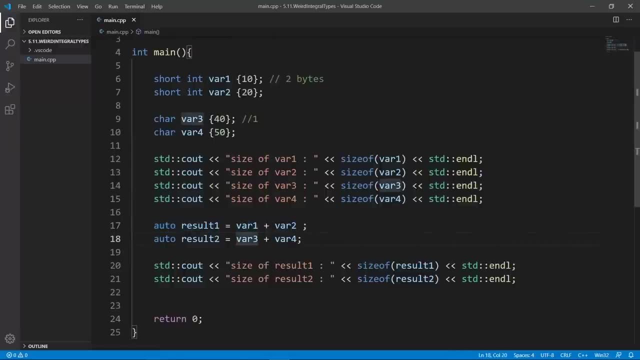 and car is going to take up one byte and we're going to print their sizes. we're going to see them printed out and we are adding things up here. we are taking two short and variables and adding them up. so what the compiler is going to do, it's going to take this, turn it into an end and then 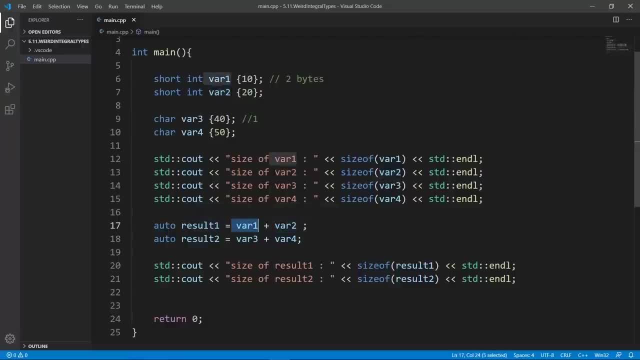 do addition and the result is going to be an end. the same story is going to happen for result two. var3 is a car, so it is one byte in memory, but the compiler can't really add up integral types which are smaller than four bytes in memory. so what is going to happen? var3 is going to be. 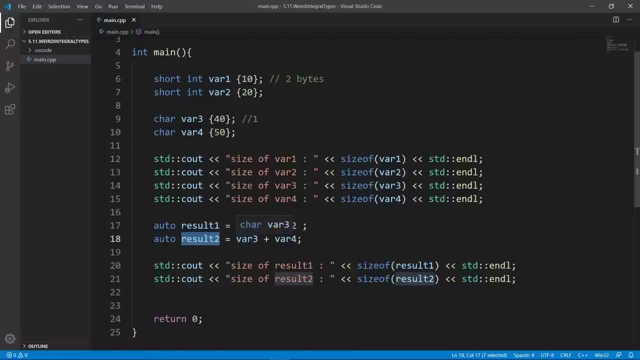 transformed implicitly behind the scenes to an end and var4 is going to be transformed to an end, and then we're going to add that up and we're going to store that in an int variable, which is result. here, if we print this up, we're going to see that size of result is going to be. 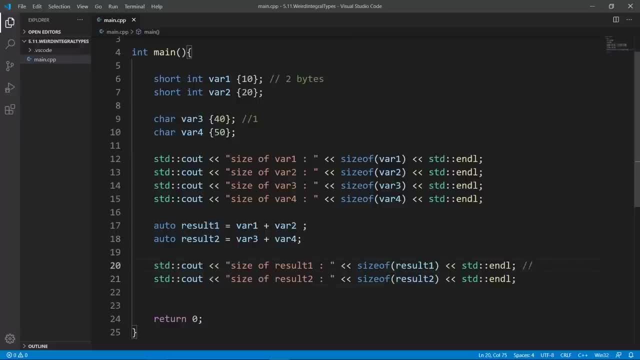 result one and result two is four, and this is what we expect here, and this is a behavior you need to be aware of, because sometimes your application logic is going to depend on the size of data. if that's the case, you need to care about this, and if you don't know this, you're going. 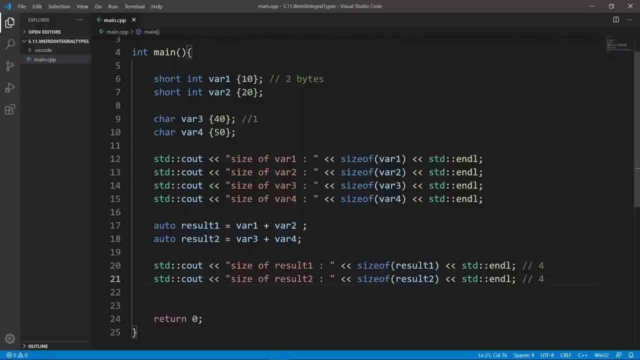 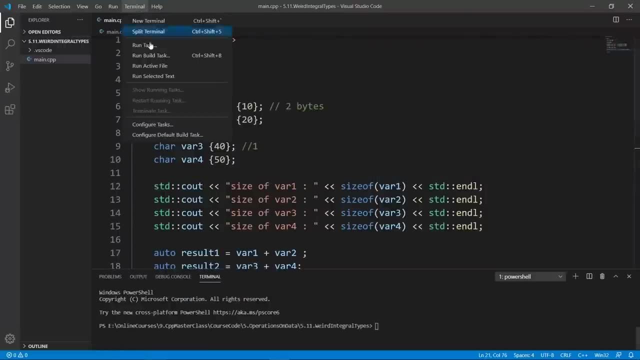 to be beaten by this, and it is really hard to find problems like this. so what we can do is open up our terminal- and we're going to build this with gcc usually do- and we can run our program rooster, and we're going to see that this is what we expect. 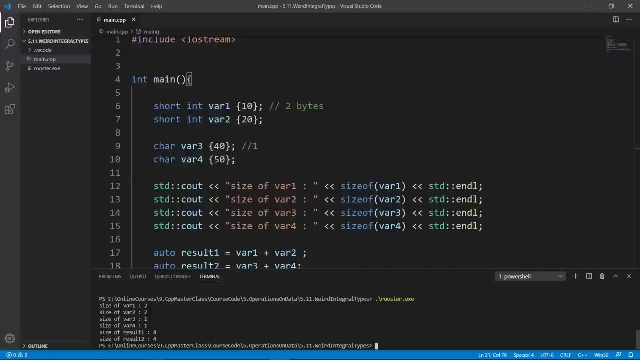 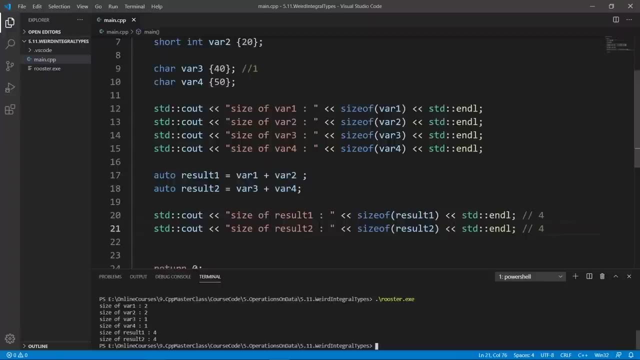 var1 is two bytes in size, var2 is two bytes in size, var3 and var4 are one byte in size, but our result is four bytes because the compiler implicitly converted our operands here to ants to be able to carry out this arithmetic operation. this is really all we set out to do in this. 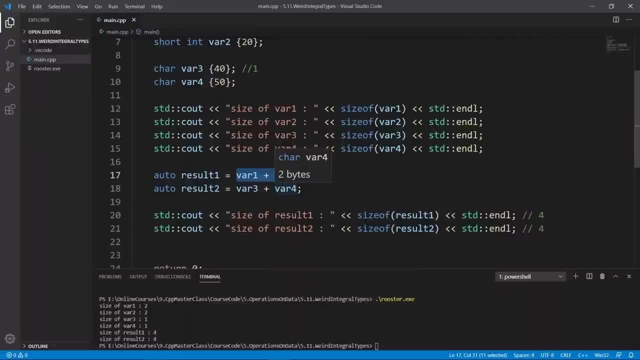 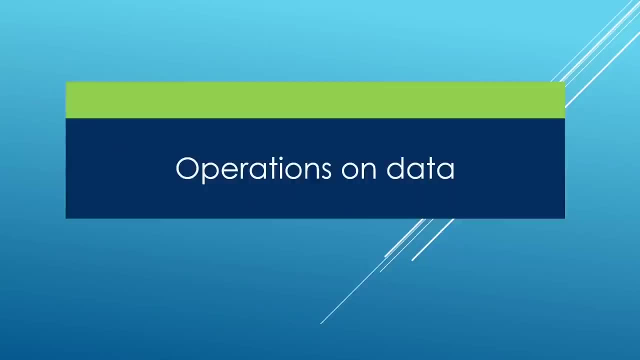 lecture. i hope you found it interesting. we are going to stop here and we're going to see you in this lecture. in the next one we're going to try and recap what we saw in the chapter congratulations on hitting the end of this chapter, and this chapter was really about. 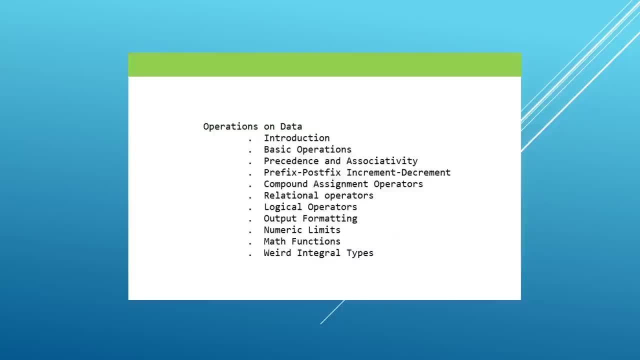 doing operations and manipulating the data that you have stored in your variables. the first thing we saw was that we could do arithmetic operations on the data. we can add things up, multiply, divide. we also saw the modulus operator, which may seem weird for beginners, but we had a chance to really play with us. after that, we learned about precedence and 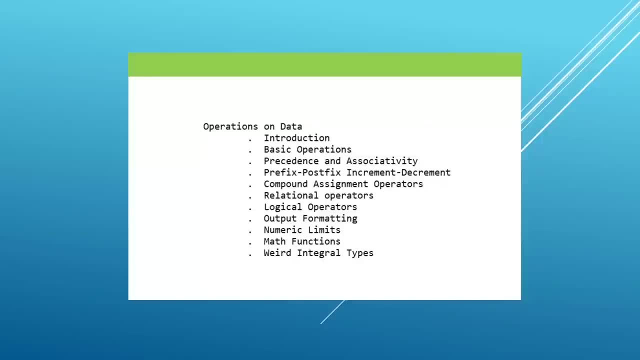 associativity. we saw that that's a set of rules we have to follow to know which operation to do first if we have multiple operators in our expression. we also had a chance to learn about prefix and postfix, increment and decrement operators. we had a chance to do compound assignments, things like. 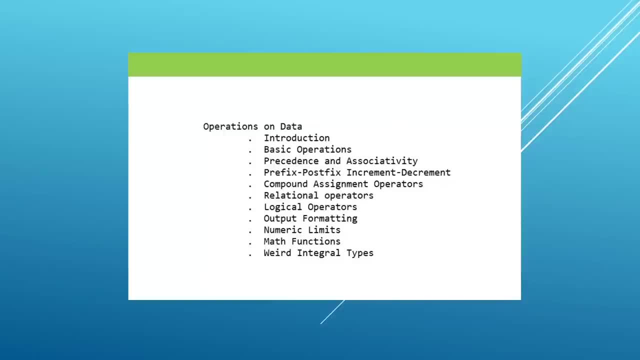 plus, equal, minus, equal, multiply, equal, modulus, equal. now these things must be making sense to you. we had a chance to look at how we could compare things using relational operators like greater than, lesser than and equal or not equal. we also had a chance to look at output formatting and we saw a host of things we could do to make data show up better with. 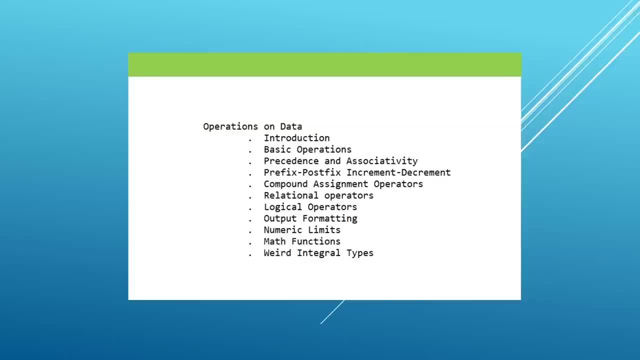 sddc out. after that we learned about numeric limits and this is a cool way to know the ranges for your data types, but there are a whole lot of other ways to do that for which we could compare with um. that's all for today and we hope that you guys enjoyed watching this video and, i really hope, the 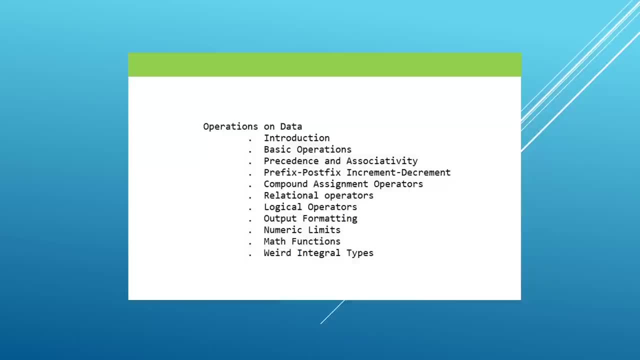 that you guys enjoyed watching this video, and that you guys enjoyed watching this video and that you host of other properties you can use in this limits library. we learned a little bit about math functions and we played with things like the power of something, the exponential, the few. 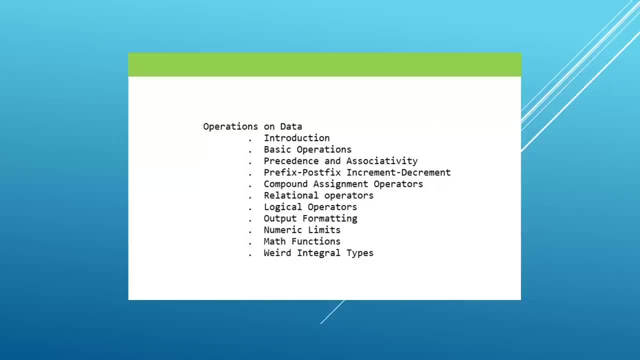 rounding functions that we have in the cmath library, and now you must have a good idea about these functions that you can use to manipulate and do math on your variables. we ended the chapter by looking at some weird integral types, and the main message in that lecture was that you can't do. 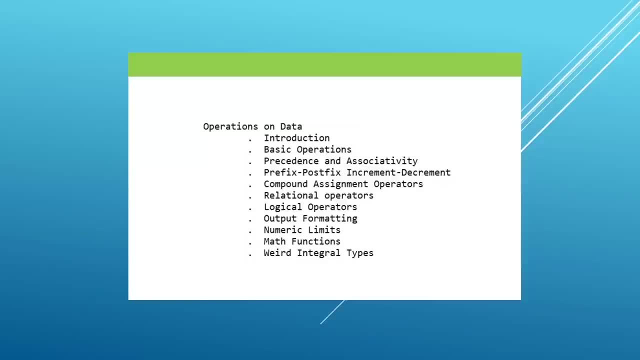 arithmetic operations on data types whose size is less than four bytes in memory. if you try to do that, the compiler is going to insert implicit conversions, and if your application depends on the size of things, this is something you need to be careful about. otherwise you're going to have 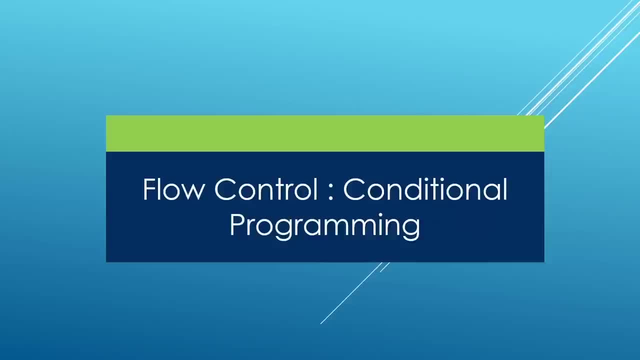 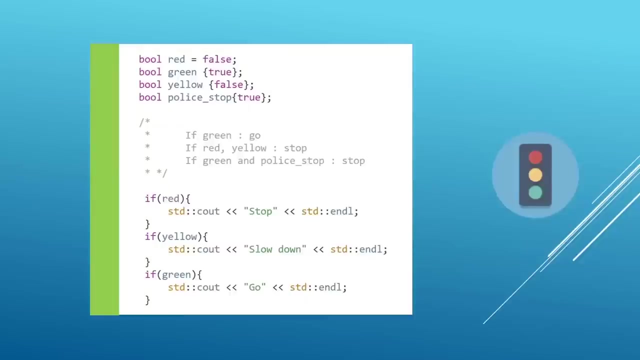 a hard time finding these problems. i would like to welcome you in this new chapter where we're going to be learning about a new way we can do things in c++ and we're going to be doing conditional programming. in other words, we're going to be able to do different things based on the conditions that we have set up in. 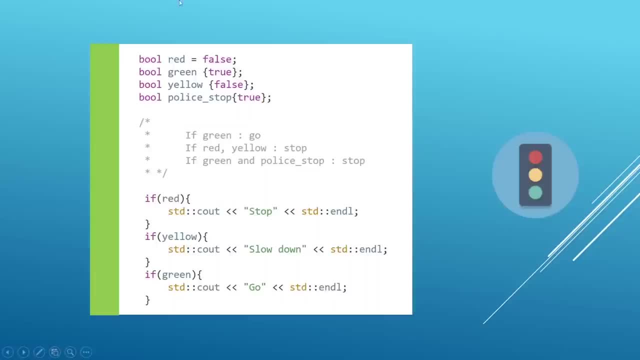 our code. just to give you an example here we have a few variables- they are booleans- and we have a few initializers in there. red is false, green is true, yellow is false, police stop is true and we can do different things based on this boolean conditions. for example, if the light is red, 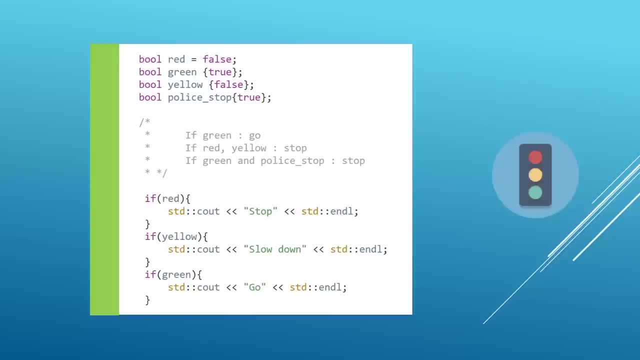 we may be told to stop. if the light is yellow, we might be told to slow down. if the light is green, we might be told to go and do whatever it is we want to do. so we're going to be able to do these kinds of things, and c plus plus provides different constructs. 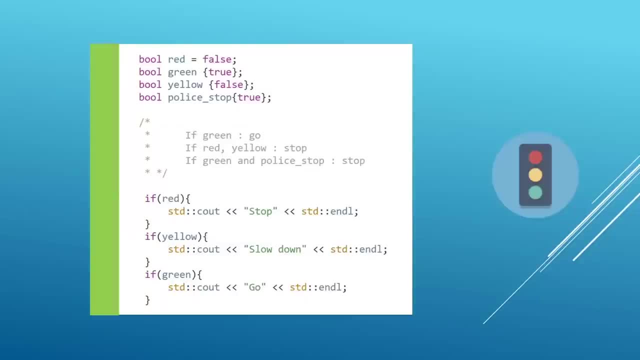 practice to be able to do conditional programming in your c plus plus code. we just have one thing to do, One of them in this slide, which is this if statement. here, this if keyword allows you to do things like this. We have a few others: We have the else keyword, We have the switch keyword. 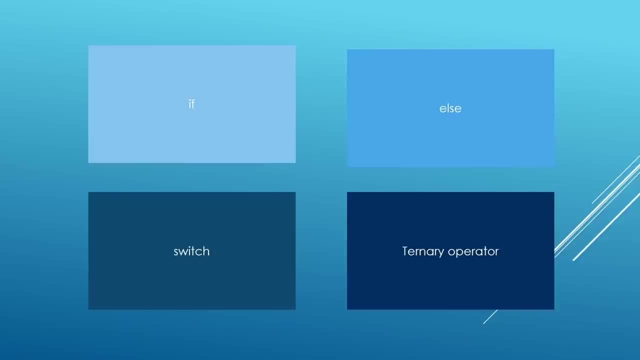 We also have a completely separate operator that is called ternary operator that allows you to do these kinds of things, And we're going to be learning about all these things and more in this chapter. We are going to start and learn about the if statement in this lecture. 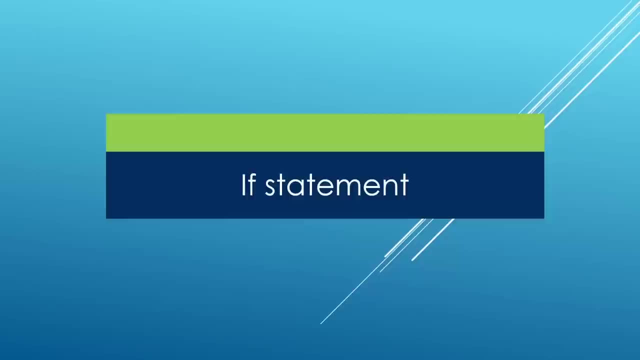 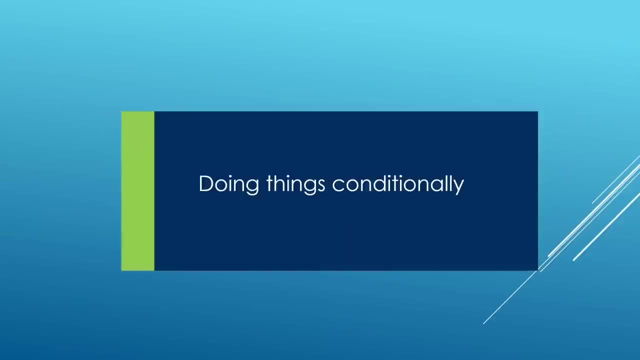 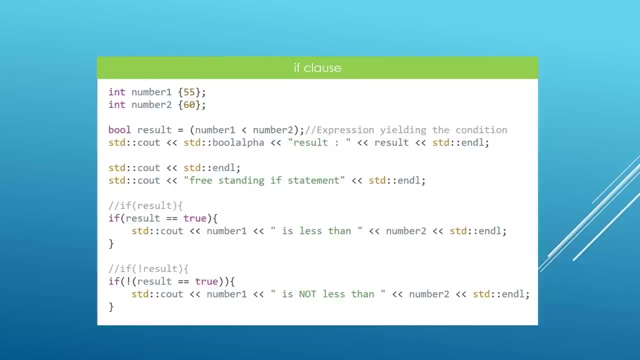 Go ahead and finish up here and meet me there. In this lecture, we're going to learn about the if statement, And this is a statement that is going to allow you to do things based on some condition being true or false. Here is a simple code example. We have two variables, number one and number two. 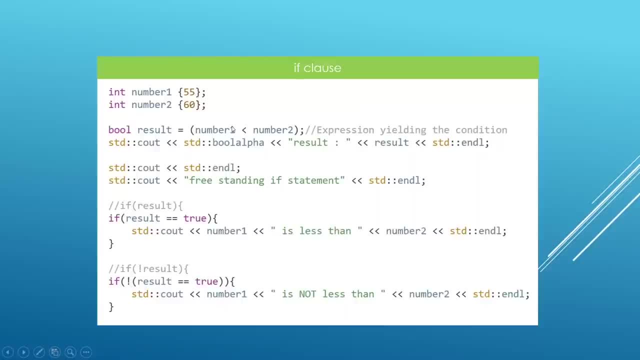 And we have a statement here that is going to compare number one and number two And we're going to store the result in this Boolean variable That we have on the left. Then we're going to do something based on the value that we are storing in this result here. 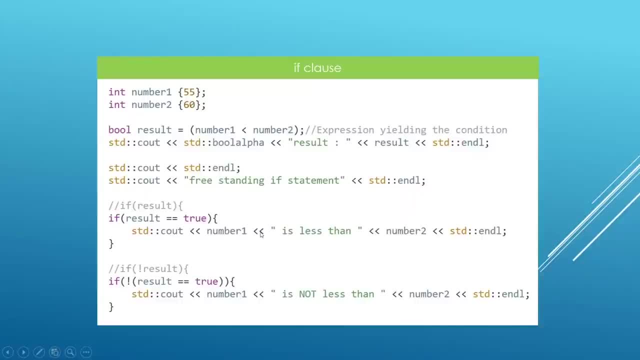 If the result in there is true, we're going to print number one is less than number two. If the result is not true, we're going to say number one is not less than number two And notice in the first if clause: here we are testing for the case where the result is true. 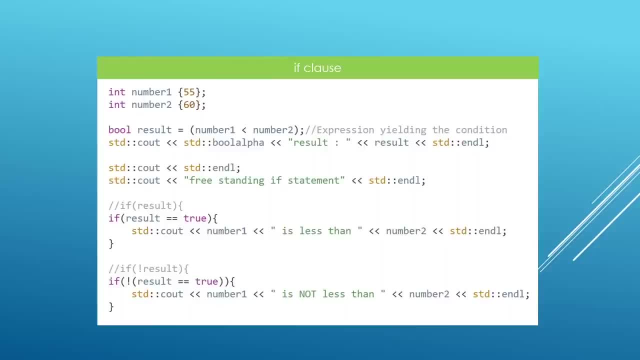 But sometimes we need to do something When this Condition here is not sure. One way to do that is to negate what we have here inside the if parenthesis And test for the reverse of whatever we have in here, If that is making any sense. 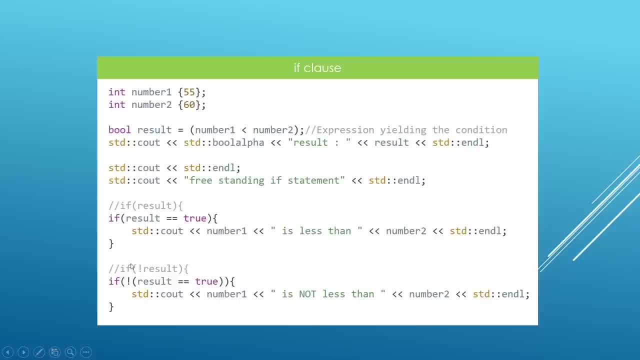 If you look here, we are testing for the case where, if not, the result is true. And in other words, we are testing for the case where the result here is false And we're going to say number one is not less than number two. 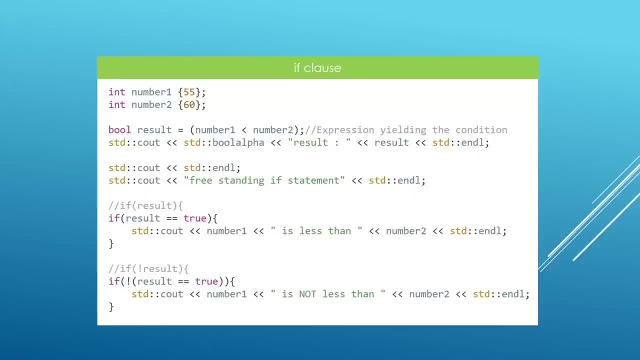 This is one way we can go about this. Again, the if statement is used to do conditional programming. This is the syntax we use to do it in C++. We say if we put the set of parenthesis, and inside the parenthesis we put the condition we want to test for. 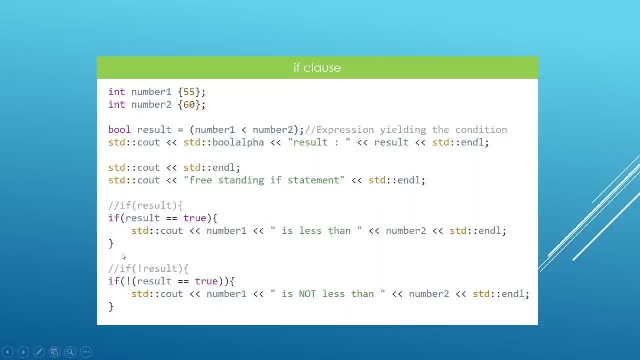 And after that we're going to have a pair of curly braces And what we have inside these curly braces is going to be the body of our if statement, And it is basically going to be the code we want to run if the test here is: 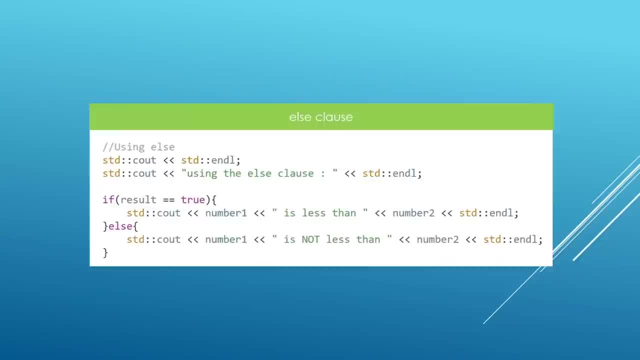 Successful. We can also use an else clause to catch the case where the test hasn't been successful. In this case, we can say: if result equals, true we're going to do something, And else we're going to do something else. 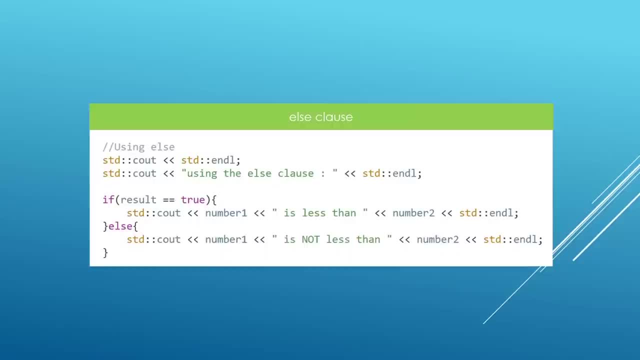 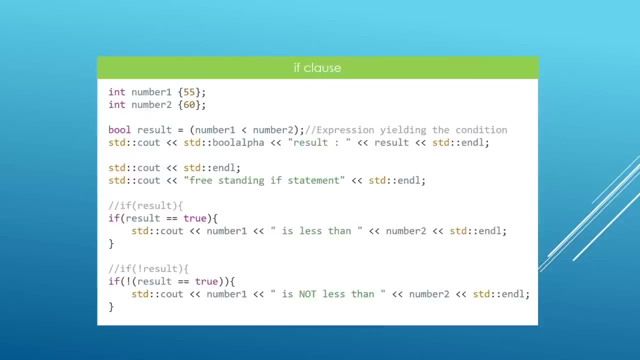 In other words, if result is true, we're going to say is less than. If it's not true, we're going to say is not less than. And this is a more compact way of doing what we just did in the slide here. 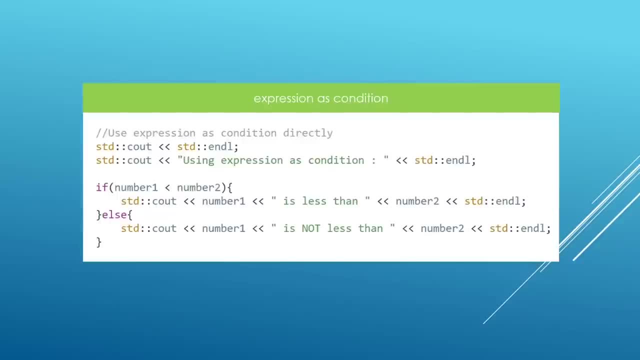 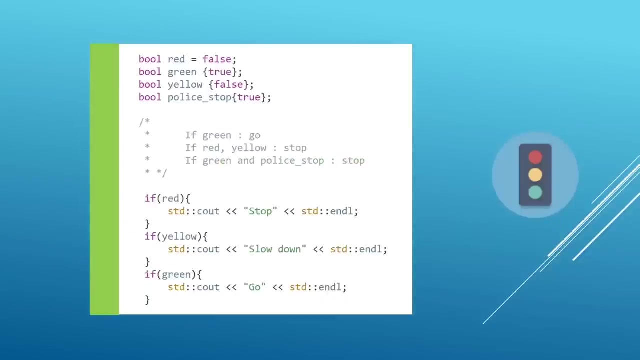 You can also directly use your expression As a condition, And the requirement here is that the expression evaluates to something that we can treat like a Boolean, Because the condition has to be a Boolean, It has to be true or false. Okay, here is another simple example. 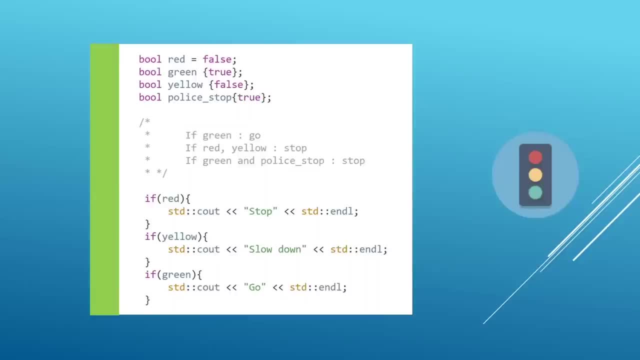 We have seen this in the last lecture. We have a few variables containing our conditions And we are saying if the light is red, for example, we're going to do something. If it's yellow, we're going to do something. If it's green, we're going to do something. 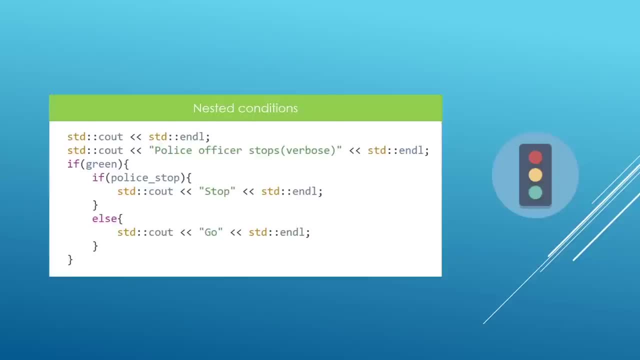 We can also nest conditions. For example, we can put our outer if statement And inside that if statement set up other if statements. And if our logic needs something like this, you can do this And you can take advantage of this to achieve whatever it is you want to do. 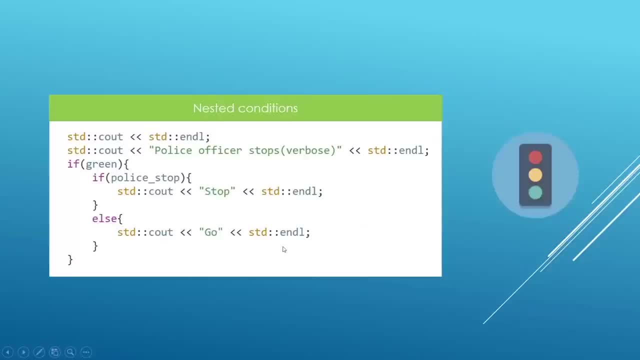 In this case, if the light is green, we're going to fall in here And we're going to do another condition. So if the light is green and if the police officer has stopped you, you're going to stop, And if they haven't stopped you, you're going to go because the light is green. 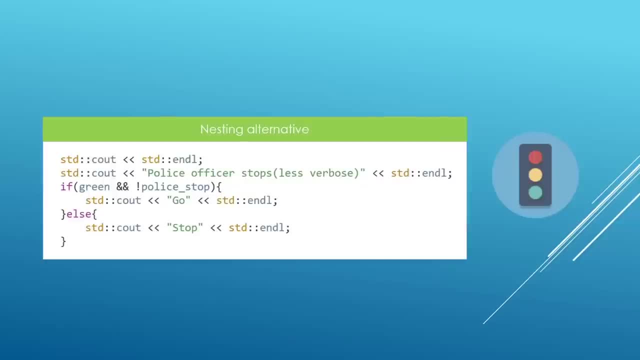 And you can do something like this. We can also use logical operators to kind of achieve the same thing And we say: if the light is green and the police officer hasn't stopped you, you're going to go, Else, you're going to stop. 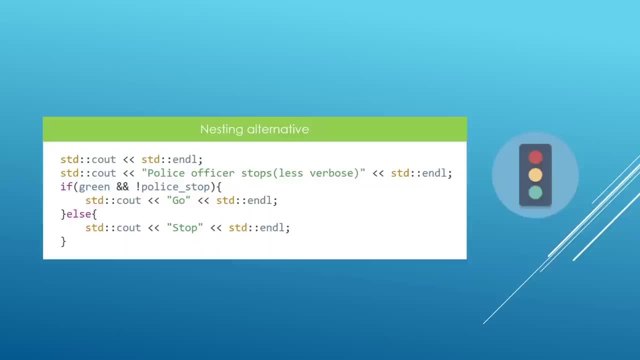 And you can do something like this And you see that you can combine the logical operators we've learned about with the conditional programming techniques we are learning about here to do really well, And we're going to be doing this all over the place in the course. 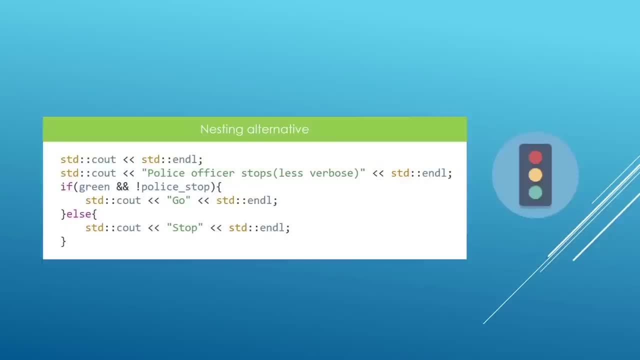 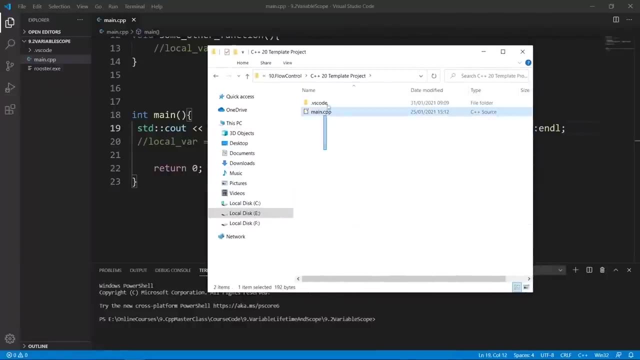 So we're going to head over to Visual Studio Code and play with us. Here we are in our working directory, We're going to be working on if statements And we're going to grab our template project, the template files, I should say. 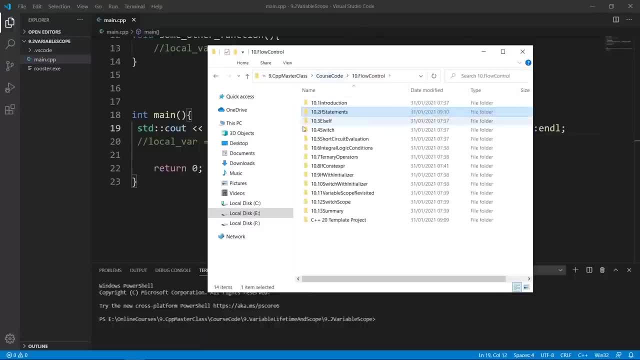 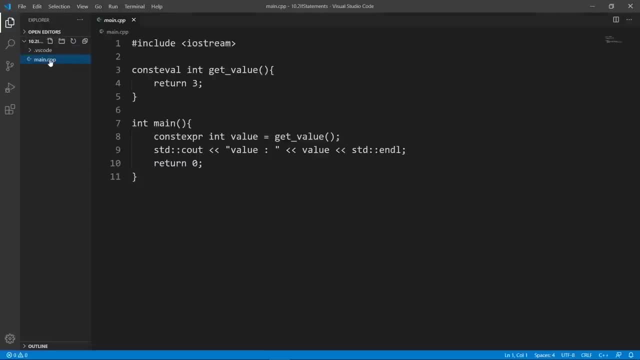 And we're going to put them in here And we're going to open this up in Visual Studio Code, as we always do. So let's do that Open folder And we should fall in here And open our main CPP file. Let's do the usual and remove what we don't need. 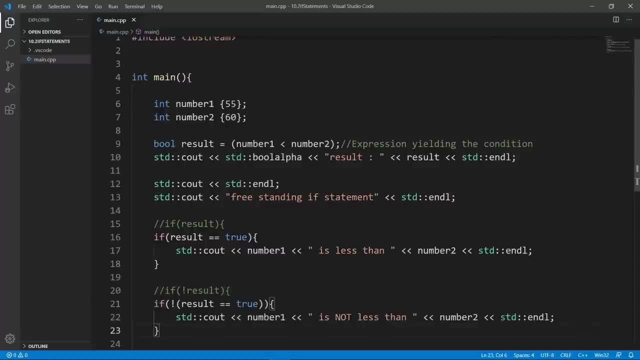 And we are going to put in our code so that we can really play with us. We have two variables in here, Number one and number two. They are integers And we have the values 55 and 60 inside. We can do a comparison between these two variables. 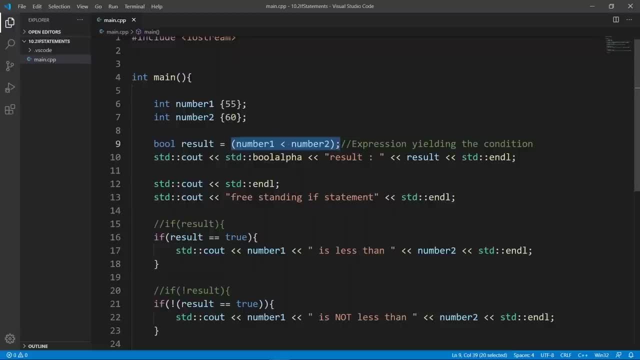 And what this comparison is going to yield is a Boolean value that we're going to store in our Boolean variable here, which is It's called result, And what we can do is use this to do some conditional programming. So we're going to say, if the result is true, we're going to do something. 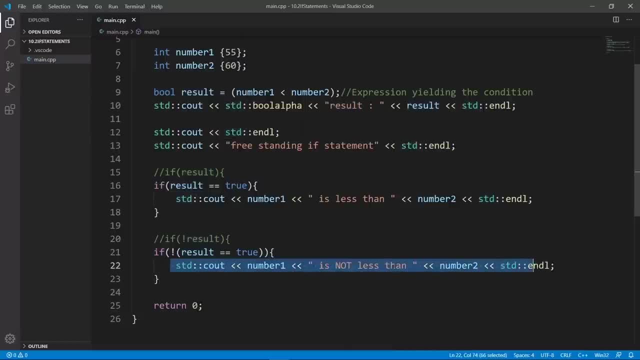 And if the result is not true, we're going to do something else, And this is how we say it. This syntax here may be confusing to new students, but try to think of it. If not, research is true, And that's really the same thing as saying if the result is false. try to spin this in your mind a little bit. 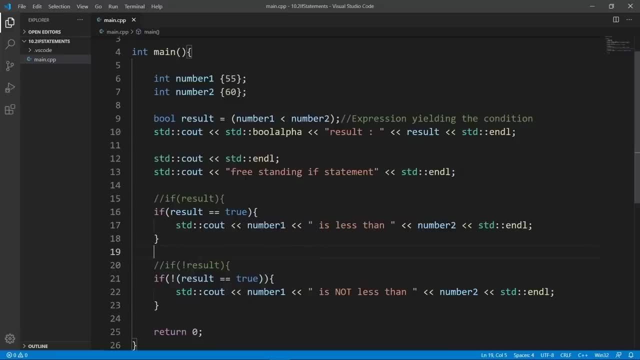 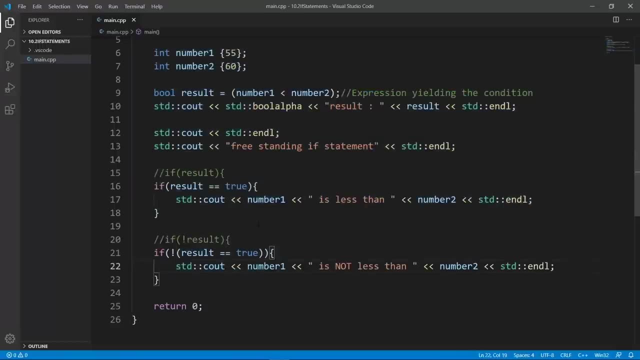 Try to spin this in your mind a little bit And you're really going to understand, OK, so now that you have seen this piece of code, try to guess what we're going to see if we run this. What are we going to see on the console? 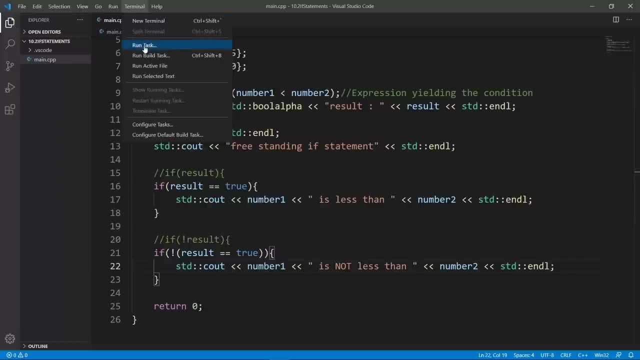 OK, give it a try. So we're going to run this in Visual Studio Code. Let's open up a terminal first, And we're going to build with GCC, as we always do. We're going to bring this up a little bit so that we have some breathing room. 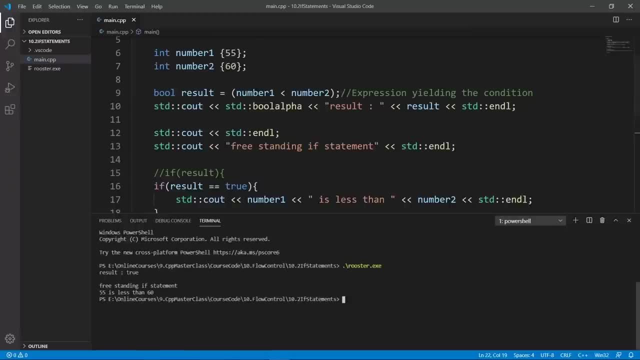 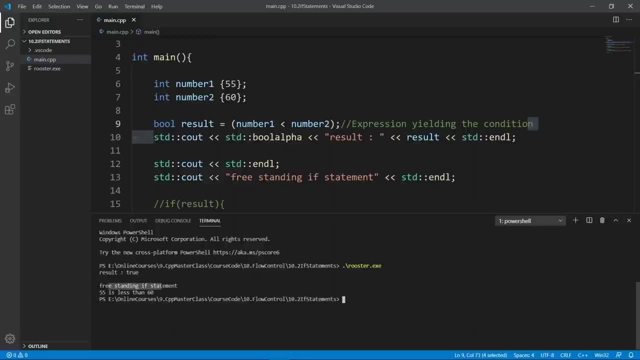 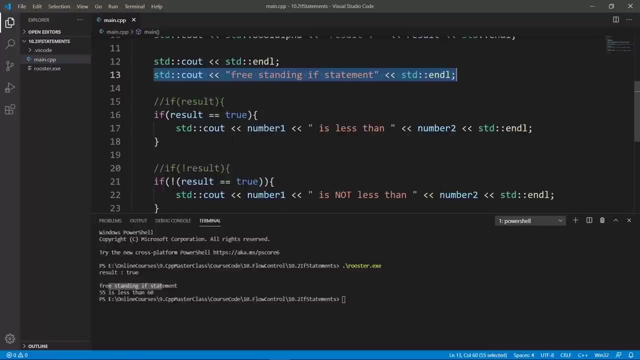 And we're going to run Rooster. Let's see what we have here. We have result equals true, And that's coming from this statement here, And we have freestanding if statement, which is coming from here, And we have our meat of this program, what we really are interested in. 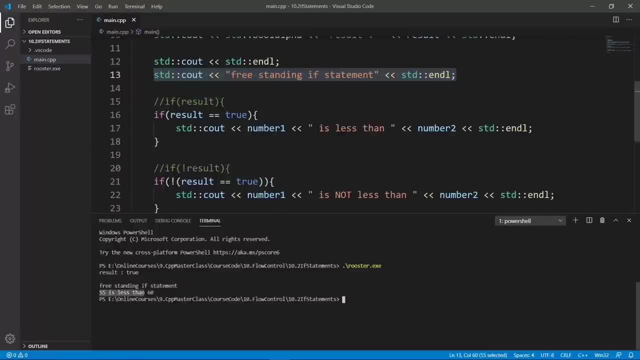 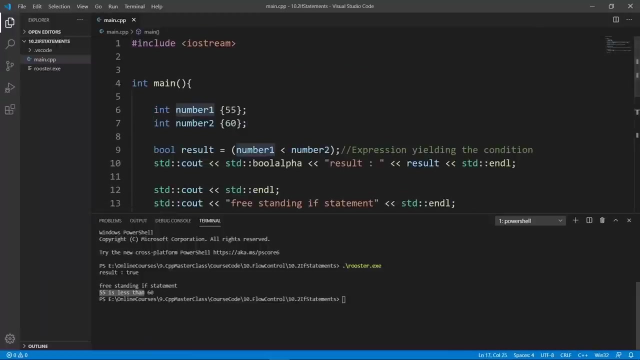 We have, 55 is less than 60. So our test here succeeded And we fell in this body and executed this stdcout statement. That's why we're saying number one is less than number two And number one is 55, which is what we see here. 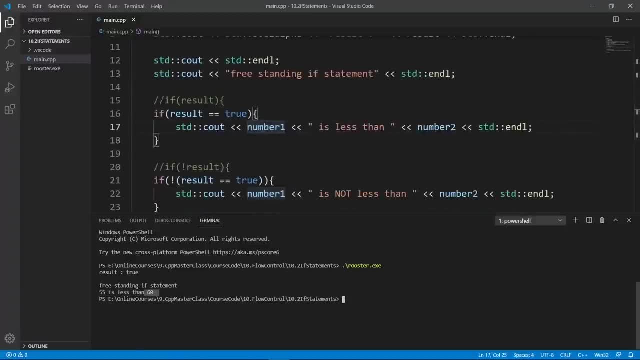 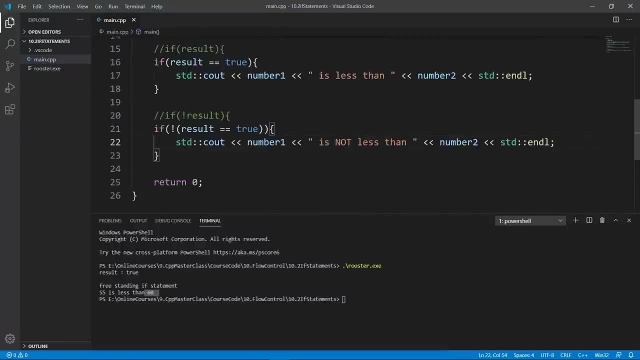 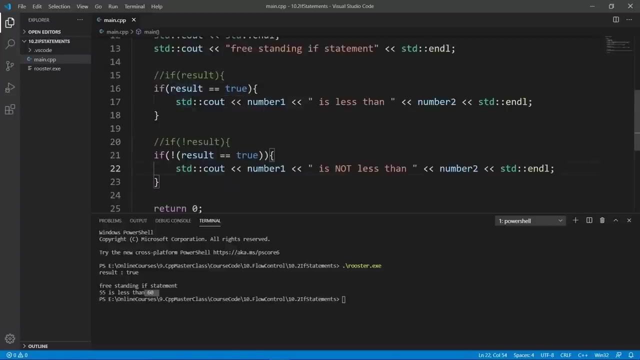 And number two is 60, which is what we are seeing here. So what can we do to make the second statement here execute? You know it is testing for the case where not result is true. So it's going to exactly do the reverse of what this test here is doing. 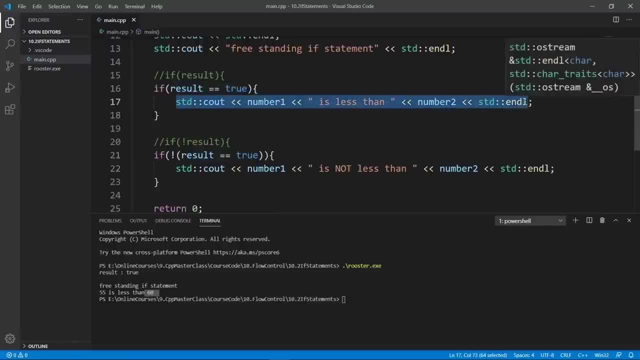 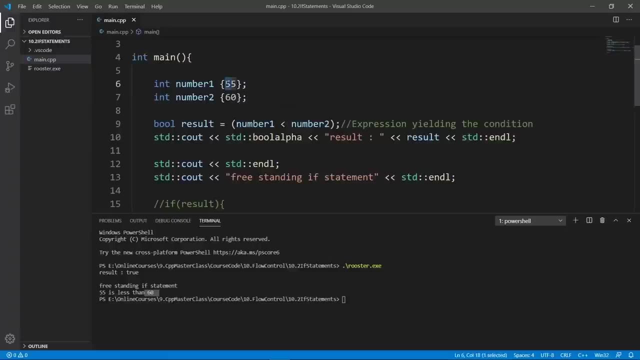 And if this fails, this one is going to succeed, which is what we have now. So what we can do to really play with this, we can go up and change this. Let's enter, for example, number one to 65.. 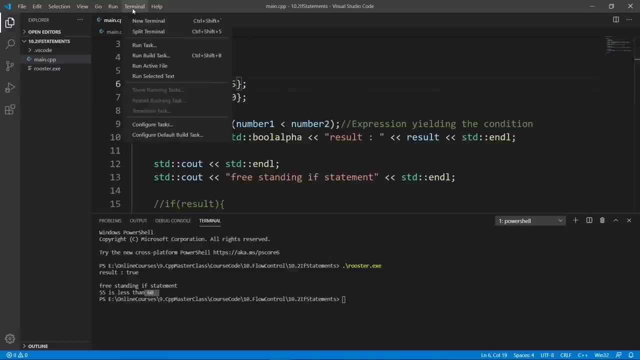 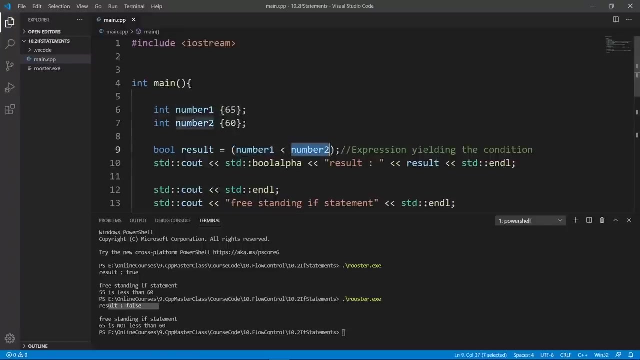 This is going to flip the order of these numbers, if I may say it like that, And if we run it- we're going to build with GCC and run this- We're going to see result is false. So result became false because number one is not less than number two. 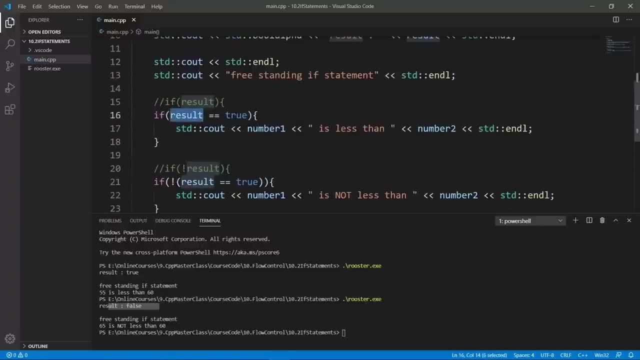 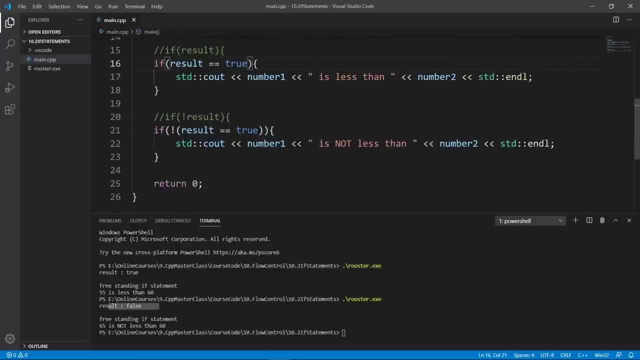 So this is going to be false And the test here is going to fail. Result is not true, So we're not going to go in here And look at here. If not, result is true. So result is true is false. 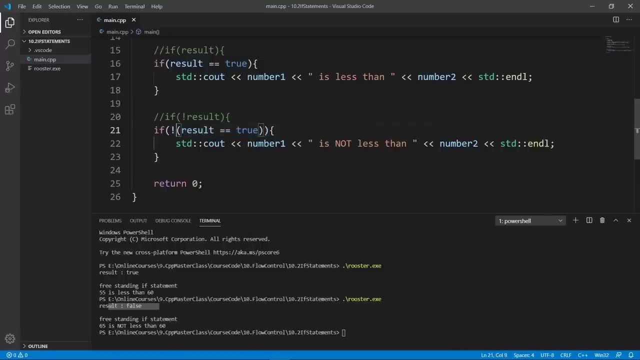 If we negate this, this is going to become true And this test here is going to succeed And we are going to fall in here. Take some time to really understand this And if you have a problem, ask me. I am going to do the best I can to help you out. 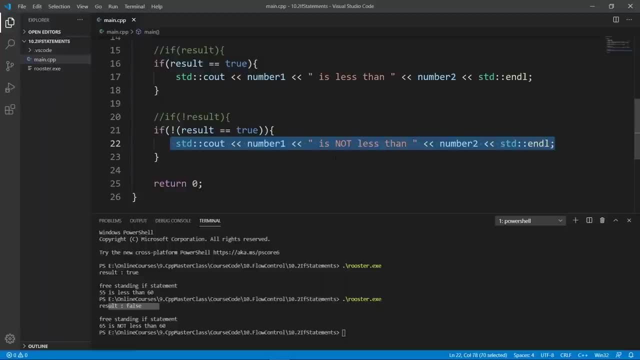 But make sure you understand this, because this is really fundamental in your journey as a software developer, not just in C++. Any career As a software developer, you're going to need to understand this. Okay, what we're going to do is comment out what we just did here, because we're going. 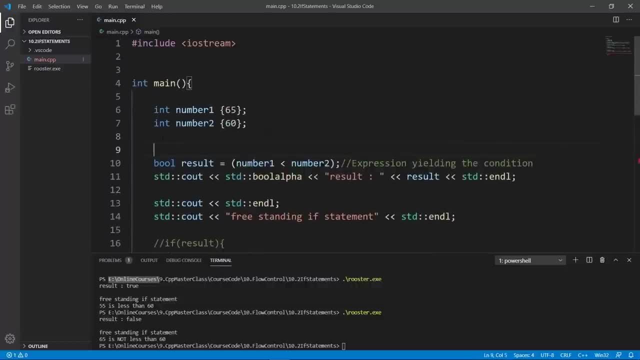 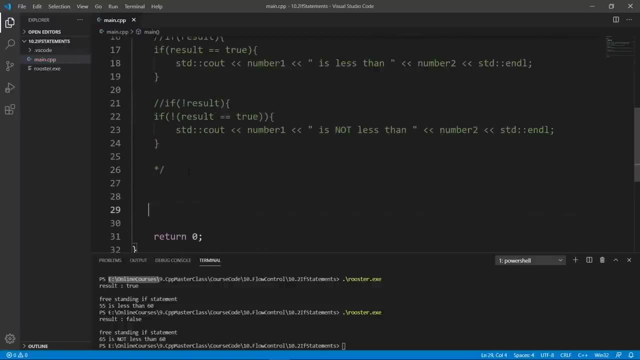 to see another way to do this, And we don't want to have noise output in our terminal. This is going to just make things hard for us to see. So what we're going to do, we're going to go down in here and put in another piece of code. 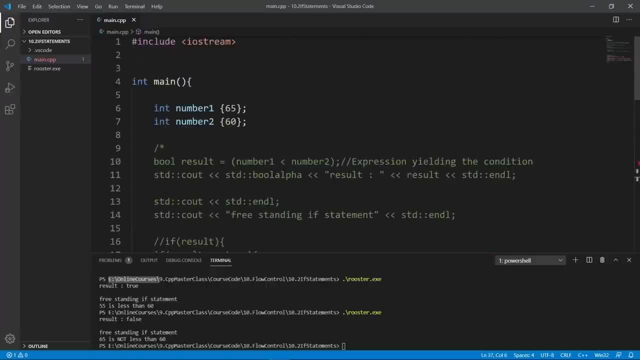 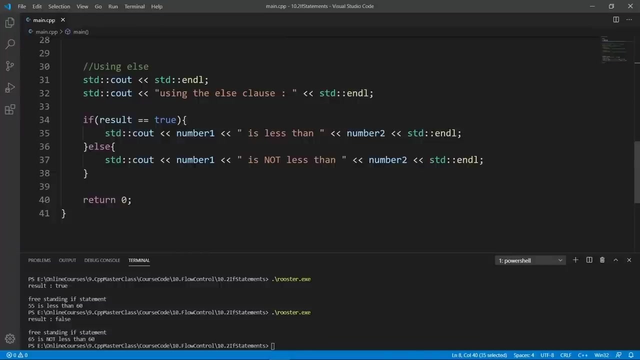 And the result was commented out. We don't want to comment that out, So we're going to take this out because this is our condition. We're going to grab it and put that outside our comment section. This is going to do, And if we go down again, we're going to click on this file icon and give ourselves some. 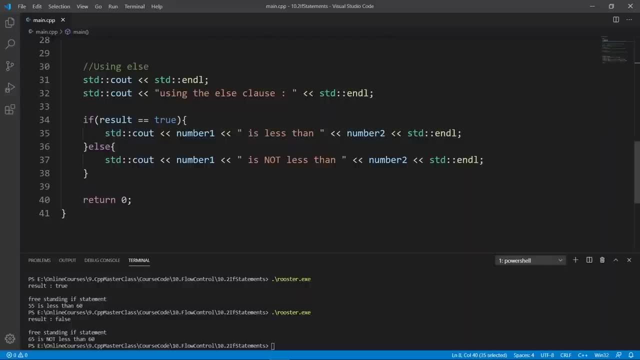 more breathing room here. We don't really need to see that main CPP file anyway. So if we come here, we can use the else close to test for the case where our condition fails. And if you look here, we are essentially saying the same thing. 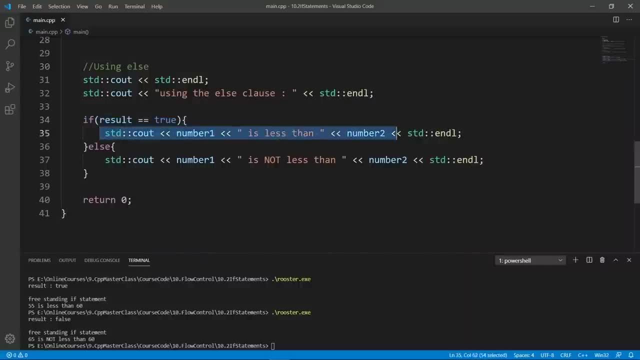 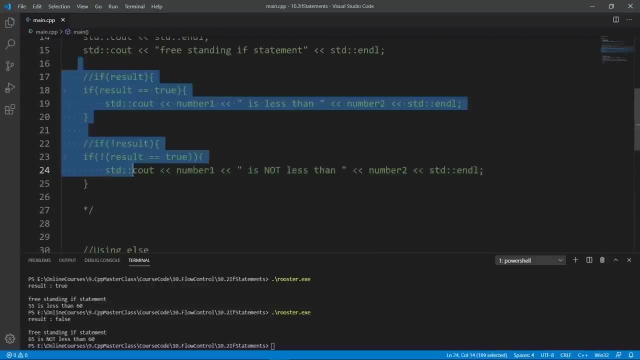 We are saying: if result equals true, We're going to fall in here, And else We're going to fall in here, So we don't need to do the double if statements that we just did here, And this is much more compact and easy to read. 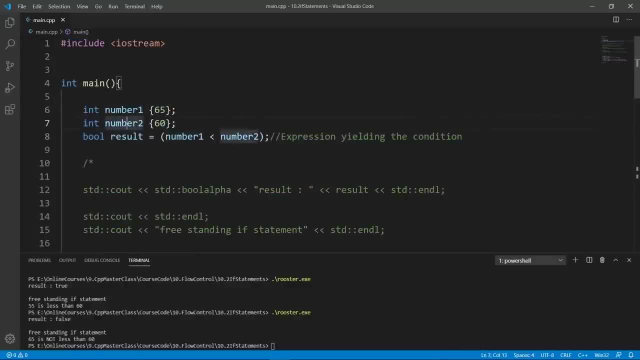 Let's look again at the numbers we have here. Number one is 65.. Number two is 60. This expression here is going to be false, because 65 is not less than 60. We're going to have a false in here. 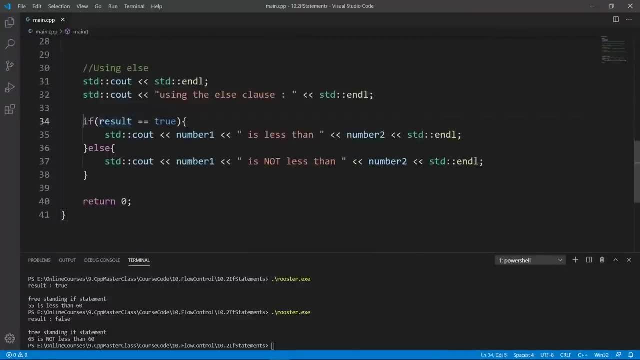 And if we come down, Resort is going to be false. This is going to fail and we are going to fall down here. We're going to Say number one or 65 is not less than 60, which is what we have in our values. 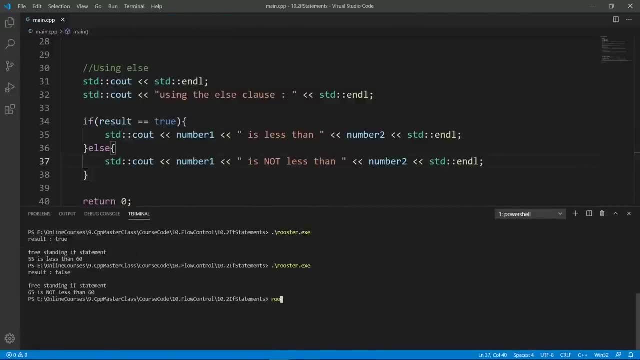 So we're going to build this again and we're going to run rooster- That's clear- so that we have some breathing room. We're going to run rooster and you're going to see that 65 is not less than 60, which is what we expect. 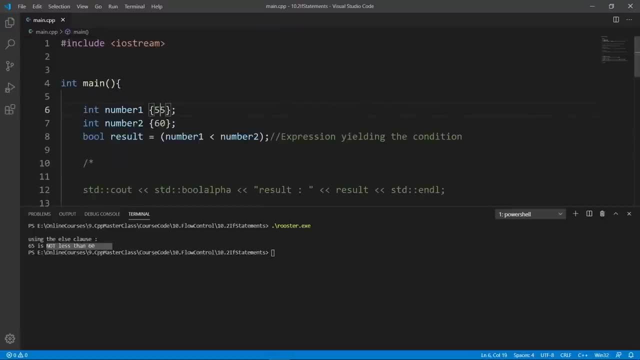 Again, if you go up and change these numbers to whatever you want, try to change these numbers to different values to see what you get As output. if we do this, we're going to see that number one is less than 60.. 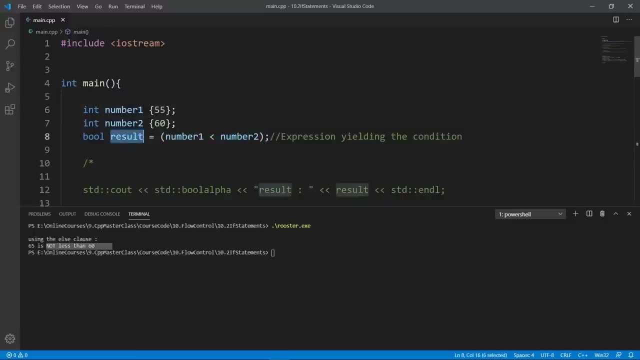 So this is going to be true and we're going to have a true in this result variable here If we go down result is true, This test condition here is going to succeed and we are going to fall in here. Let's click in our terminal and hit enter. 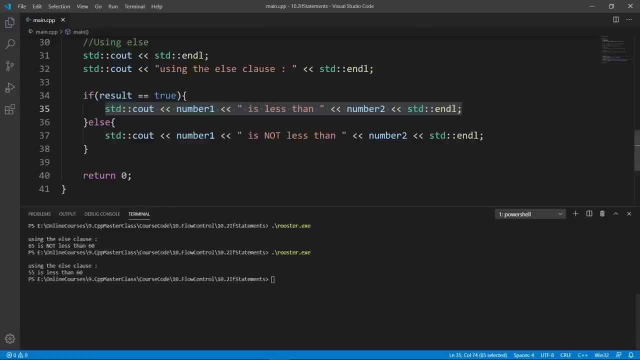 We're going to run rooster. We're going to see 55 is less than 60, which is what we have here. Okay, Now I hope you have a better idea of how you can use the else close To make your if statements really compact, and this is really cool. 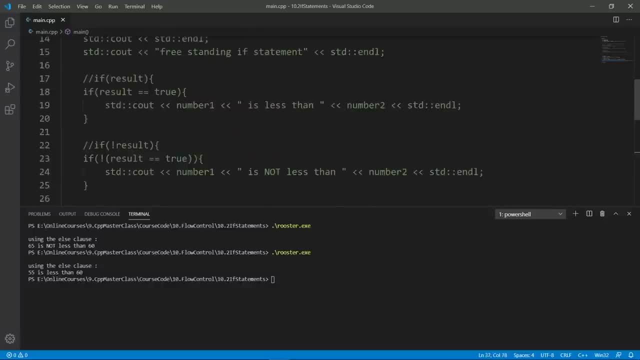 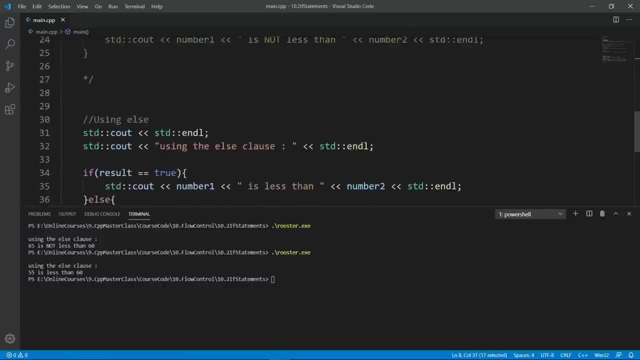 Okay, Another thing I want you to see is that you can, uh, not go through a variable like this and use an expression as a condition directly: C plus plus allows you to do this. So what we're going to do, we're going to comment out what we just did. 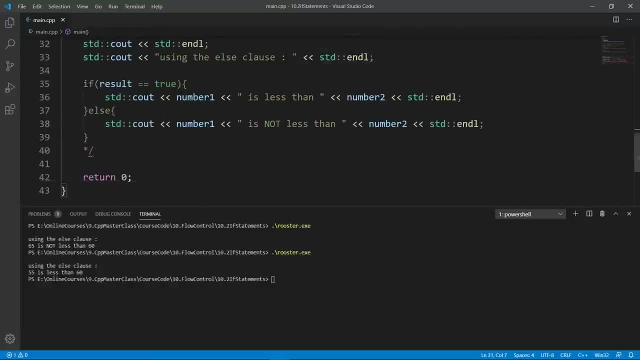 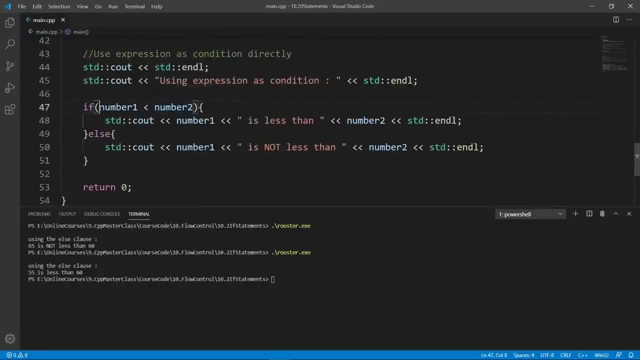 Let's do that, Going to use a block comment- I hope you know how to use this already- and we're going to go down and put in our code. It is exactly the same thing, but we took the expression and put That in the place of our condition variable here, because this is going to evaluate to a Boolean anyway. 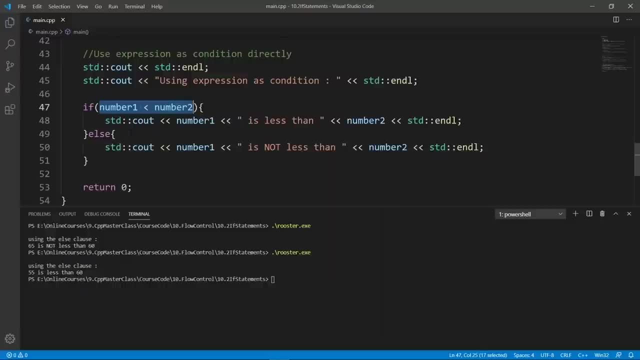 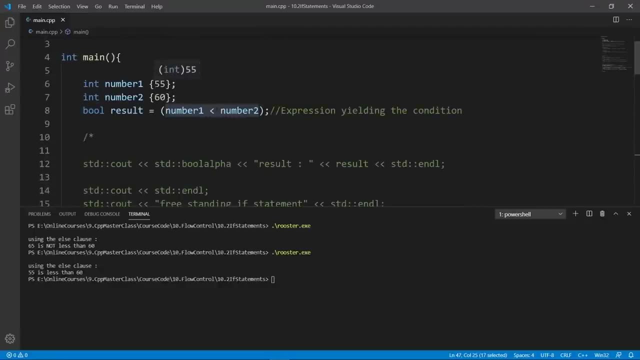 So we can use this as a condition and this is something very legal to do in C plus plus. So if we run this, we're going to see. let's see what we have in the numbers. I have forgotten by now. So 55, number one. 60, number two: number one is less than number two. 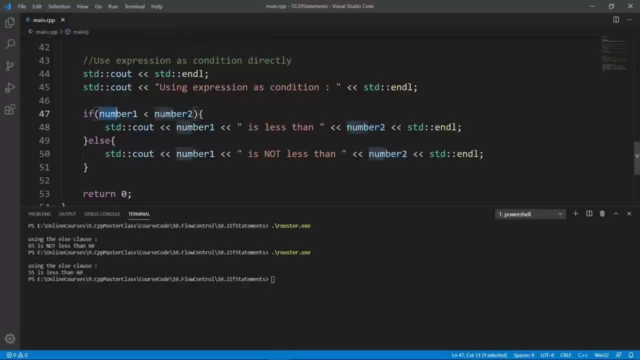 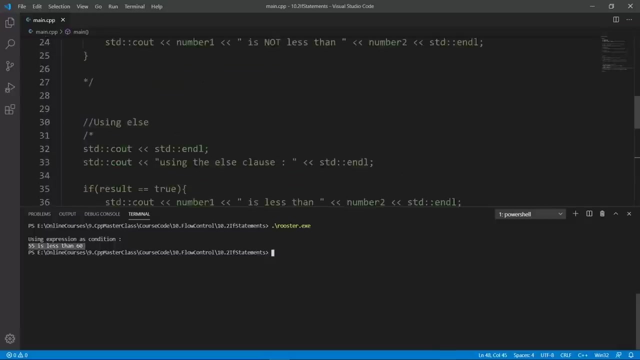 This is going to be true. So the test here is going to succeed and we are going to fall in here. That's what we're going to say. We're going to weld with GCC as usual and I'm going to clear and run rooster and you're going to see that this is the output we expect if we change up the numbers again. let's take this and make it a 75. 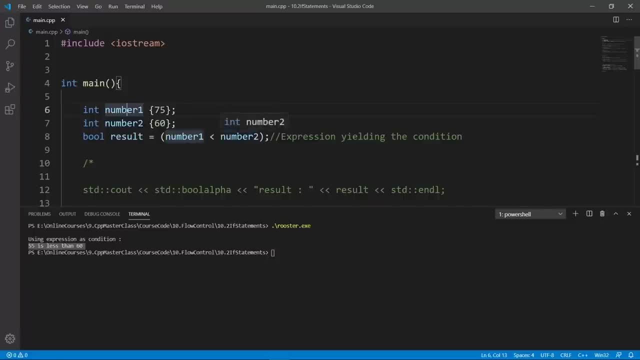 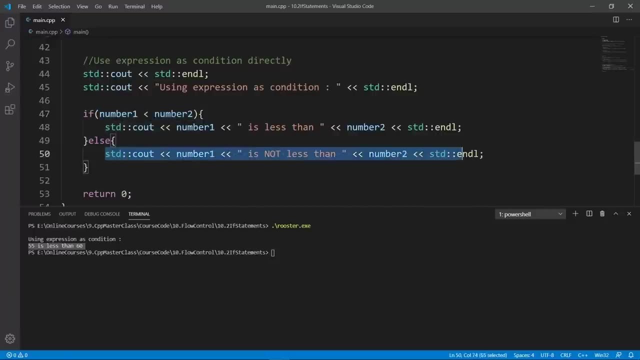 Number one. So number one is less than number two is going to evaluate to false. The test here is going to fail and we are going to fall in this block. here We're going to fall in the else clause of our test. here We're going to say: 75 is not less than 55.. 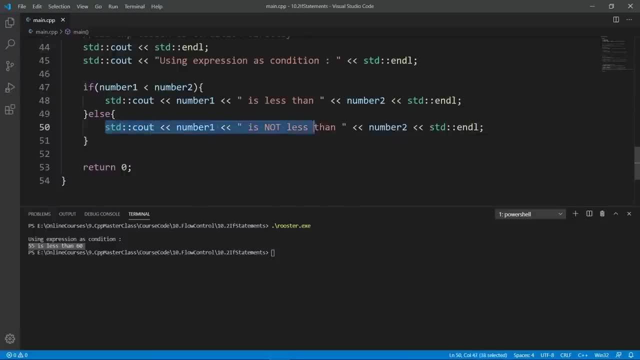 Is that what we have in there? It's a 60, but this block here is going to execute. That's the most important thing. So we're going to run this and we're going to try and clear and run rooster. We're going to get what we expect. 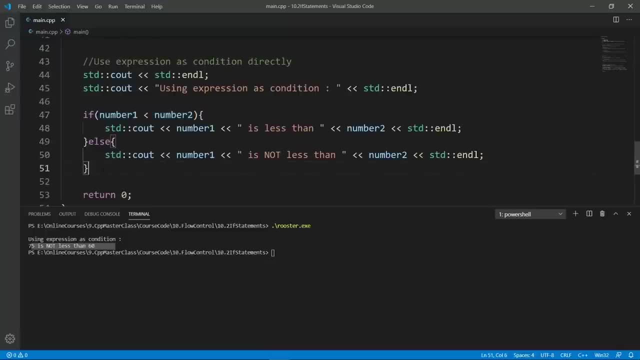 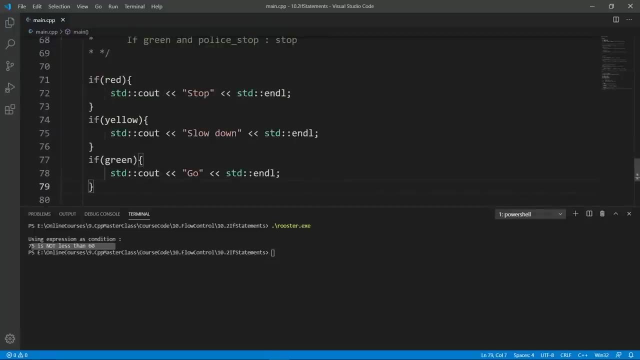 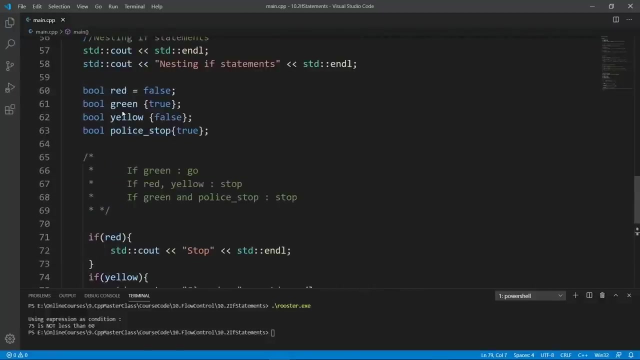 This is one way we can do this and it is really cool. Let's comment this out and see another example, And if we go down, we can see the example we saw in the slides, which was Using red, green and yellow to simulate a traffic light. 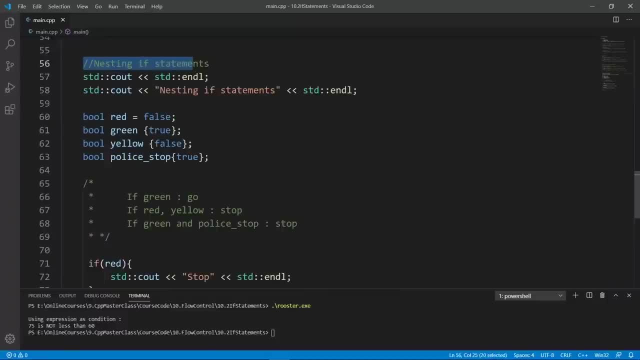 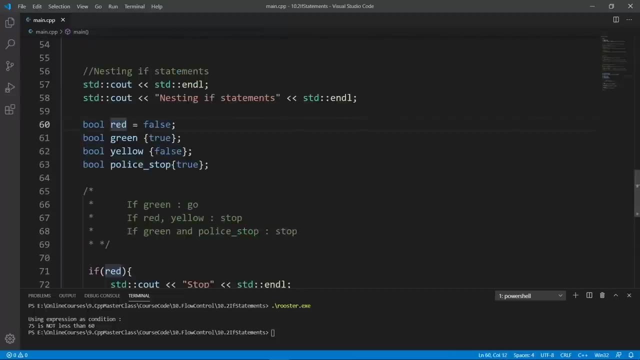 So what we really want to see here is that we can nest stuff, But before we do that, we need to try and use these conditions because it is just fun. So if red is true, meaning that the red light is on, we're going to stop. 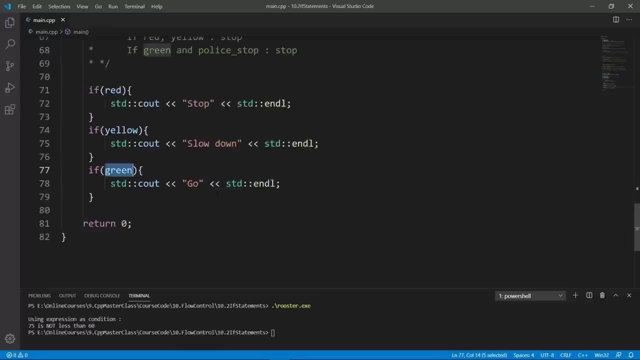 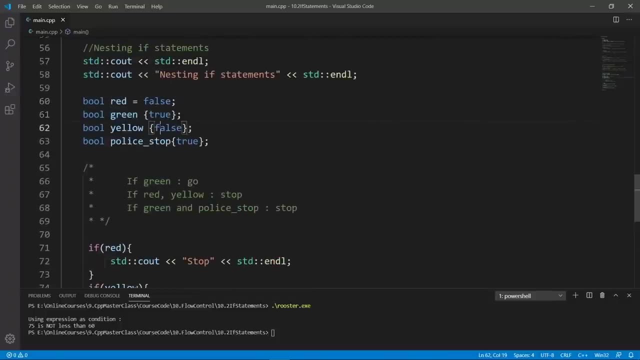 If yellow is true, we're going to slow down, If green is true, we're going to go. And if we look at what we have here, Right Red is false, Green is true, False is true And a police stop is true. 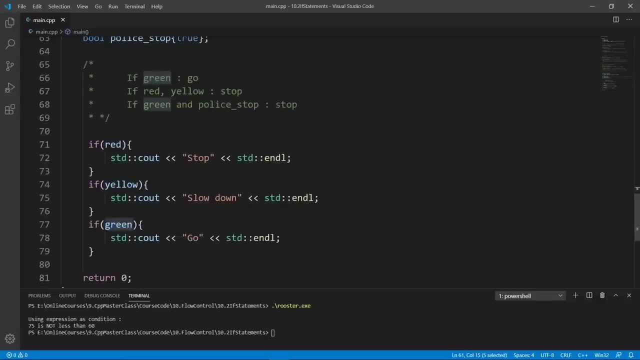 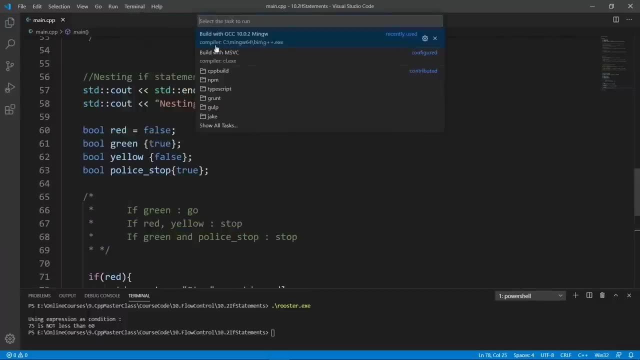 Police stop is not really being used. So green is true, We're going to execute the green statement here and we're going to say: go, That's what we're going to say, Let's try and run this. We're going to work with GCC. 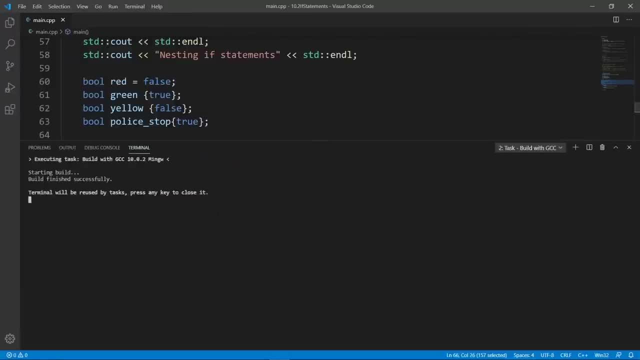 Bring this up a little bit so that we have some breathing room and we're going to clear and run rooster And you see that it is saying: go here, You can try and Change these boolean variables to different things and see what is printed out here. 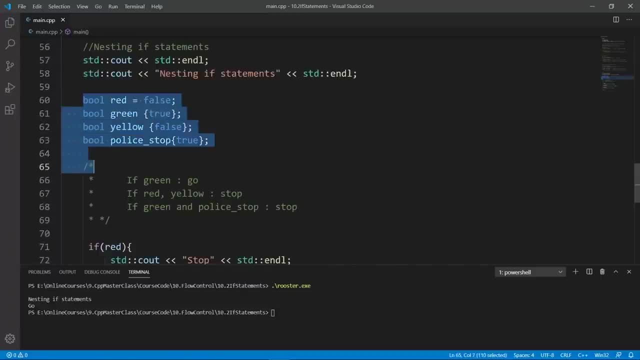 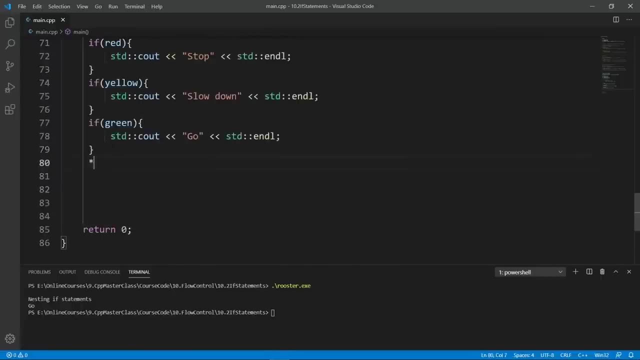 This is a great way to learn, But what we really want to try here is nested statements, And let's go down and do that, Okay, Again, we don't want what we have on top here to disturb us, So we're going to comment this out and we are going to go down and put in our code for nested if statements. 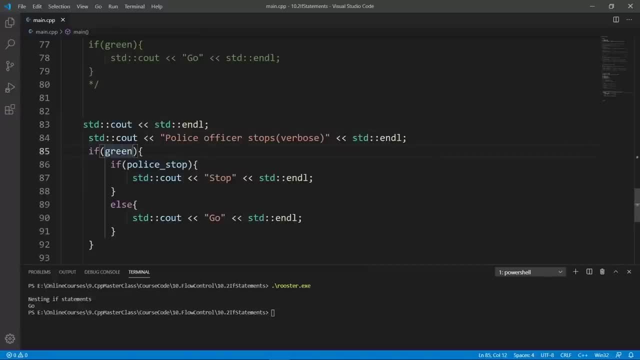 So what we're going to say Is: if the light is green, we should go, but the police officer has the right to stop us, Even if the light is green. at least these are the laws in the country where I leave. So we have a variable called police: stop here. 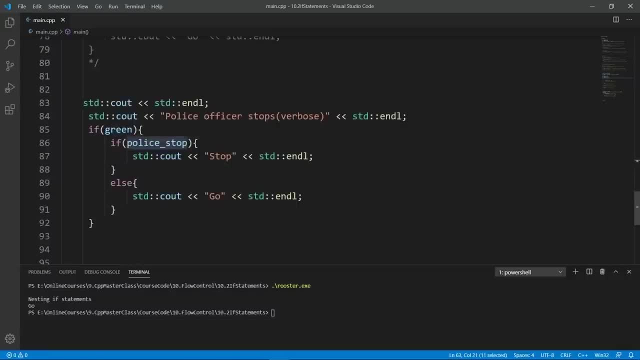 So if they stop you, even if the light is green, you're going to stop and we're going to see what we see here. So if the light is green, we're going to fall in this body again and we're going to run this inside or nested if statement. 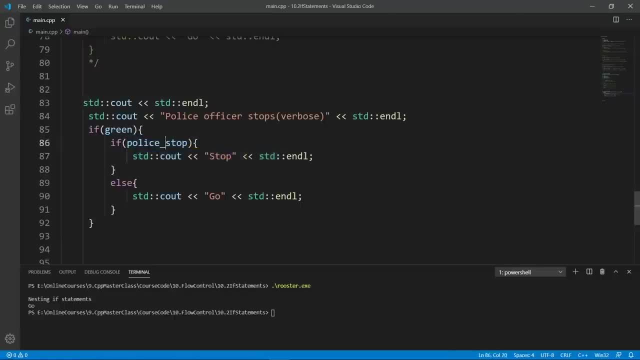 And if the officer has stopped us, we're going to stop. If they haven't stopped us, we're going to go and go on our merry way. This is what we want to see here And again. I want you to stop for a moment. 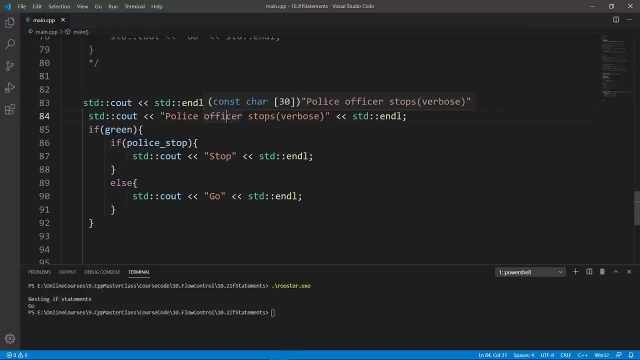 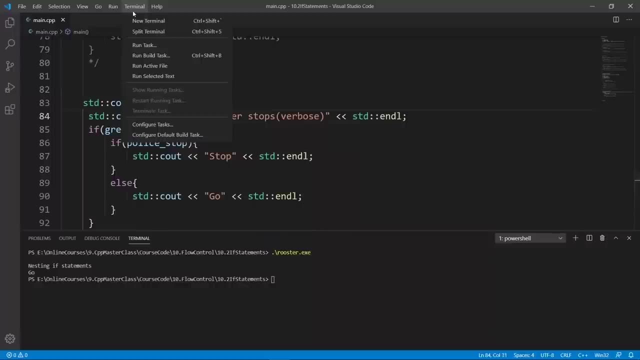 Try to run this through your brain and try to come up with the value we're going to see when we run this in Visual Studio Code. Pause for a minute. We're going to run this, We're going to build with GCC and we're going to run our program. 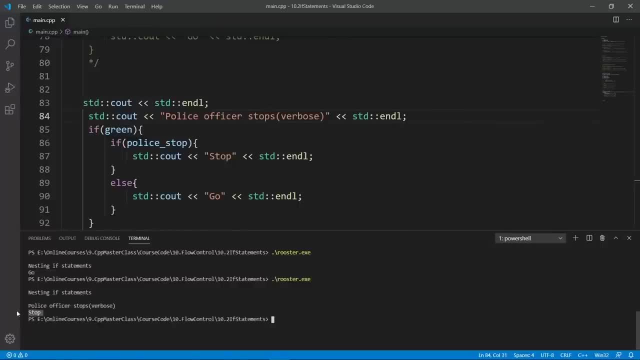 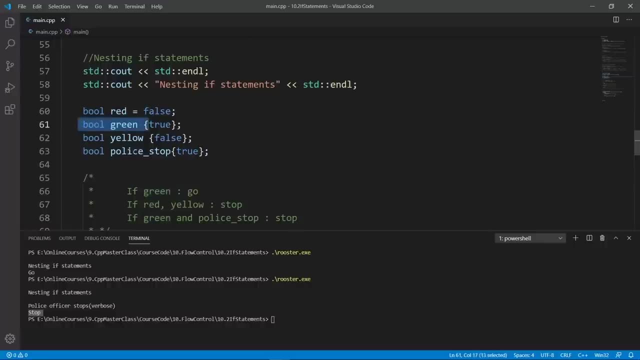 And you see that Police officer stops stop. And why is that? The light is green, OK, so we should usually go, but the police stop variable here is also true. So if we fall in here, this is going to execute and it is going to succeed and we are going to say stop. 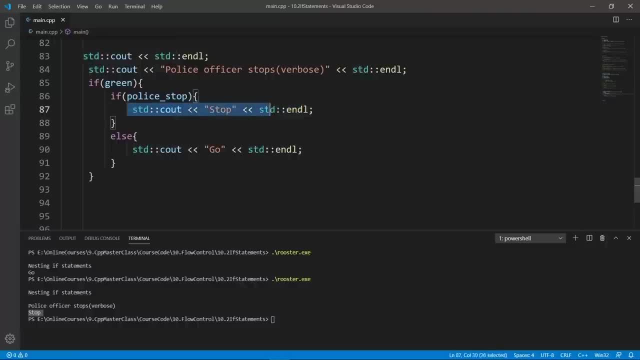 And once this statement executes, the else statement is not going to execute. Control is going to fall outside here and we're going to keep doing whatever we have Outside this if statement. here. this is really critical to understand: if one block of a nice statement succeeds, all the others are not going to execute. and try to really understand this. 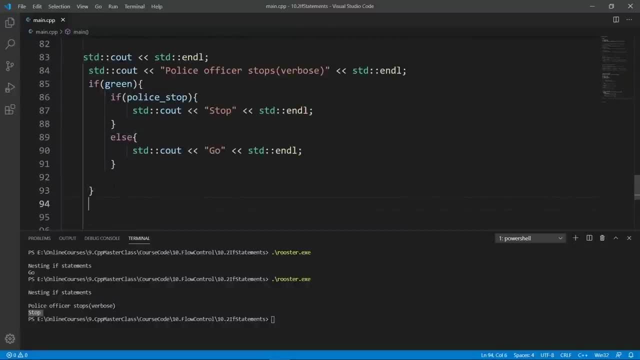 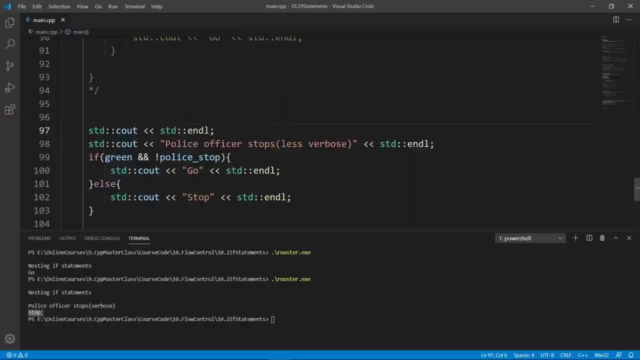 OK, we have seen this. We can now comment this out, because we have something else I want to show you. We're going to comment this out, and that's that you can combine the if statements here, or conditional programming with the logical operation. Of course we're going to do that. 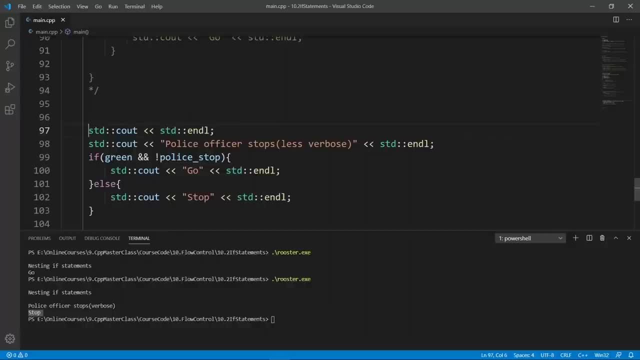 We're going to say: if the light is green and the police officer hasn't stopped us, we're going to go, and if they have stopped us, we're going to stop. and you're going to see that we're going to get exactly the same result that we had before. 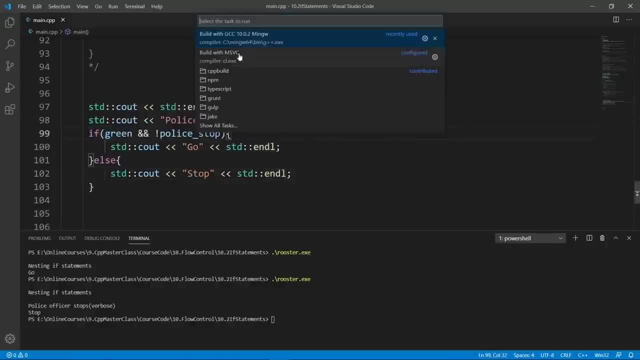 But this is really much more compact. So we're going to run and see the result of this and we're going to clear, clear and run rooster. You're going to see that they're going to stop us And this is really cool. 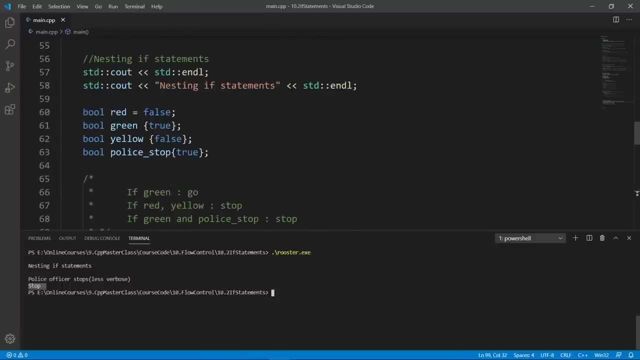 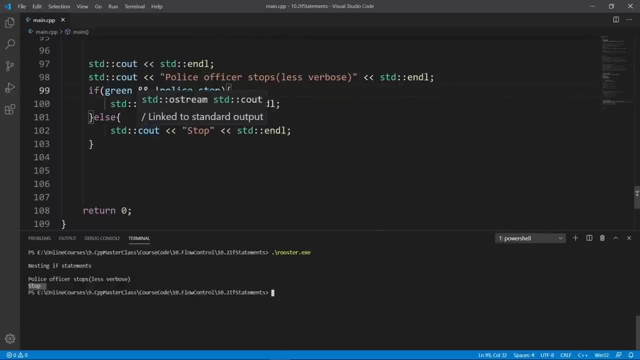 You can go up again and change up these variables to really anything you want and see what you get and try to really understand what is going on here. It is not difficult And the if statement is really fundamental to any programming you're going to do. 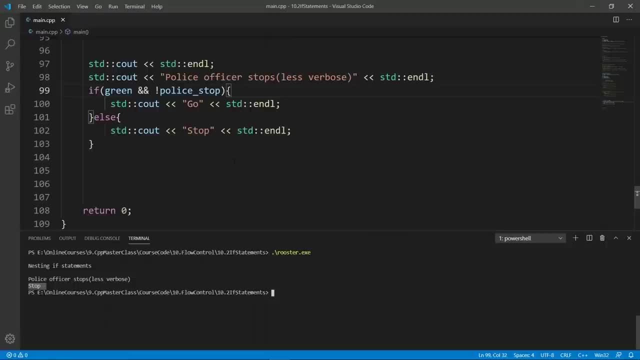 So this is really all we set out to do in this lecture: to learn about Conditional programming using the if statement. It is a powerful thing and you're going to see it all over your software development career, So make sure you really understand this. 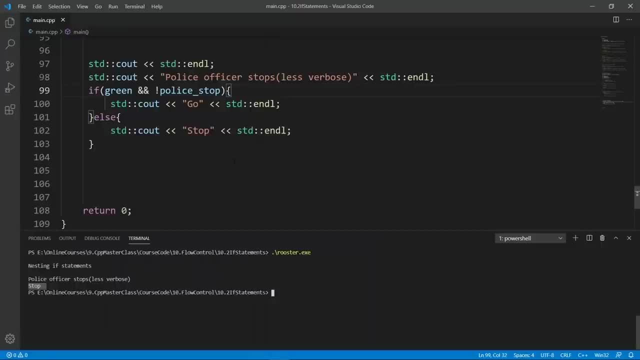 But even if it's not clear, now we're going to have a chance to do many examples and you're going to really understand what this is all about. We are going to stop here in this lecture. The next one, we're going to see how we can use the else if close. 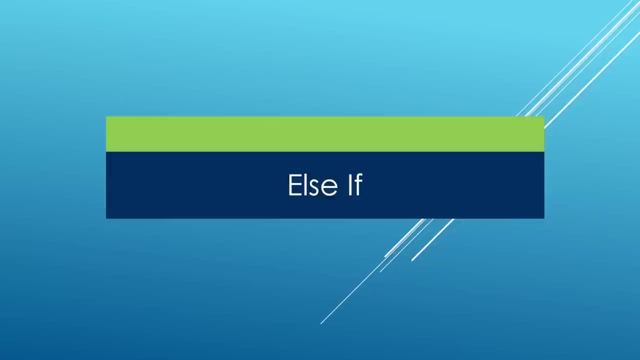 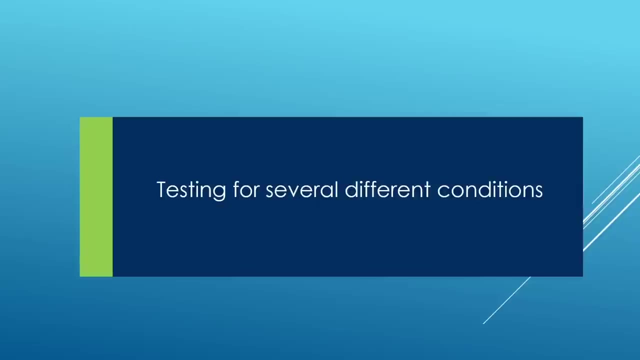 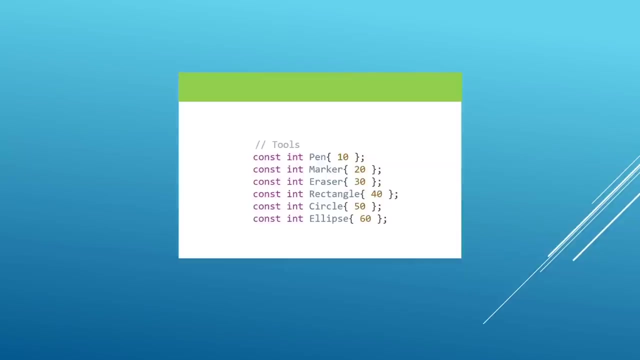 Go ahead and finish up here and meet me there. in this lecture We're going to learn about the else if close that you can attach to your if statement And that's going to allow you to test for several conditions in your if statement And to really understand this. suppose we are building a drawing application. 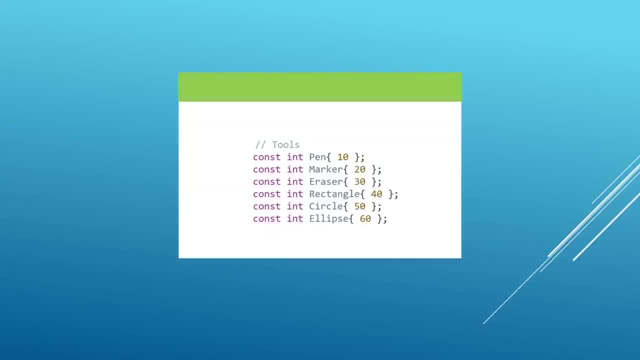 And at any given moment, the user might be using the pen or the marker or the eraser or really whatever tool that it is. we provide in our application And if we want to draw, we need to know which tool is currently selected by the user. 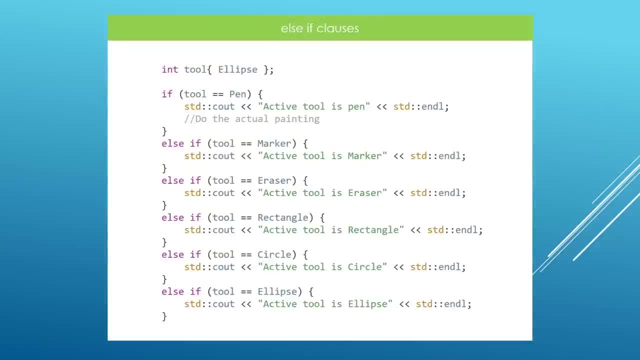 And we can do a piece of logic like this: We can have the tool storage somewhere in our application And when we get to the moment where we want to do something- for example, when the user clicks with their mouse and they want to drag and start doing things- 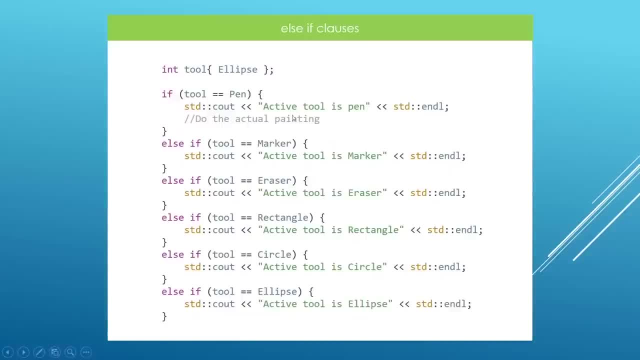 Then we're going to test for the current tool. If that is the pen, we're going to use the settings for the pen. If that's really the marker, We're going to use the settings of the marker marker and we're going to keep doing this and select one tool that is actually selected as 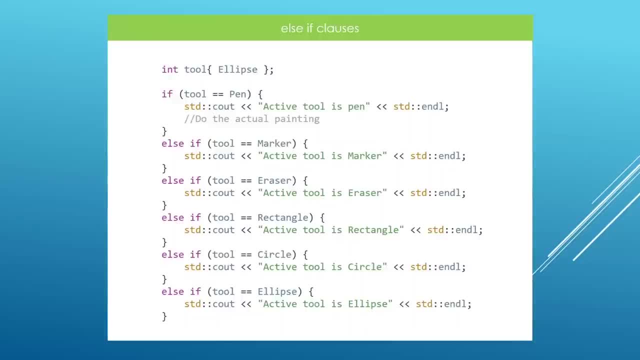 the current tool by the user. and when you do something like this, only one block in this whole chain of statements is going to execute. so, for example, if we have the marker as the current tool, the code inside this block is going to execute and say: active tool is marker, but nothing else. 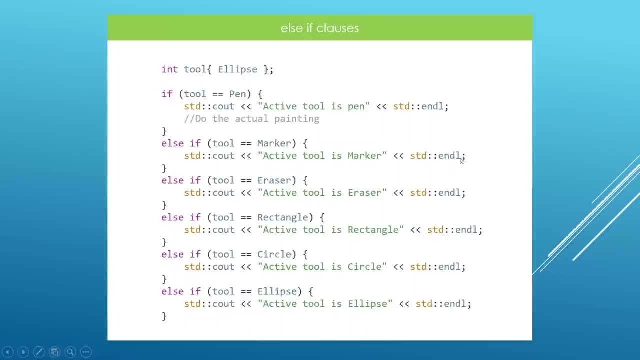 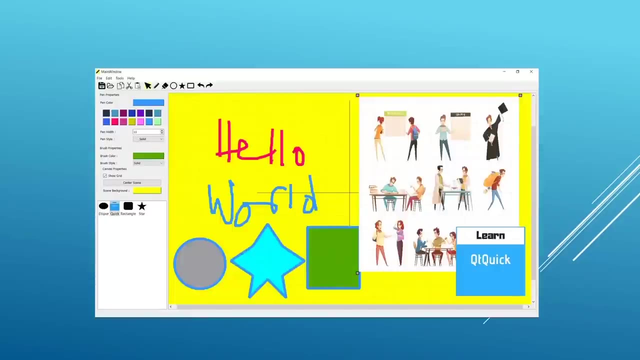 in this block is going to execute after we run. this statement control is going to jump at the end of this whole chain of if and else if statements here. i really hope you understand this and this is really powerful stuff. for example, this is one of the applications i have done in one of 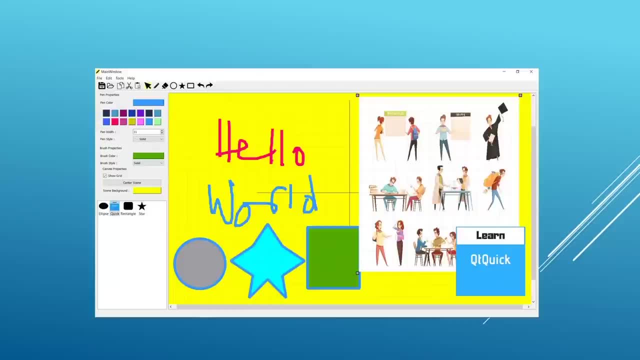 my advanced course about qt and c plus plus. qt is a framework that allows you to do graphical user interfaces like this and you can build applications like this. so what i did here is i did the exact same thing that we have here. i had a chain of if and else, if statements and whatever. 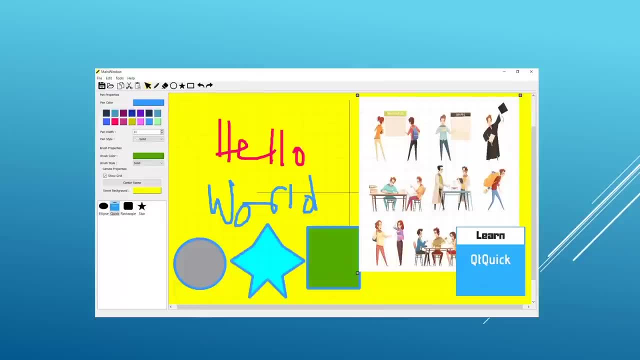 tool was selected, as the current tool was used to draw things on the canvas here. for example, if the current tool was the pen, and the pen is this little pen tool here, if it is active. we're going to draw things like hello world here if we have the star selected. we're going to draw stars if we have the 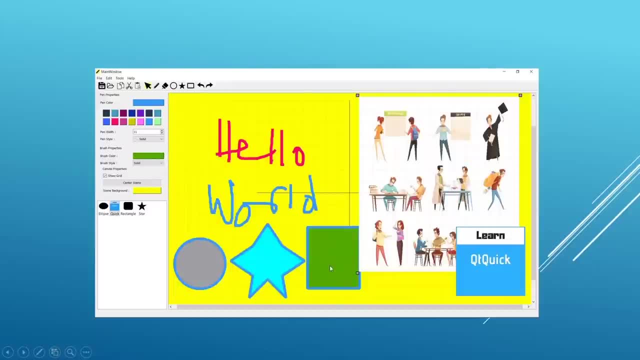 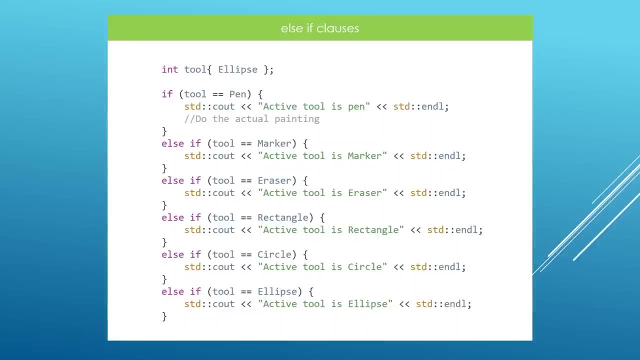 rectangle selected. we're going to draw rectangles. we could do all kinds of crazy things using this piece of logic here, and we have a lot of if statements, but it is powerful stuff and you really have to make sure you understand this. so this is how the else if clause can really help you. the main thing is to 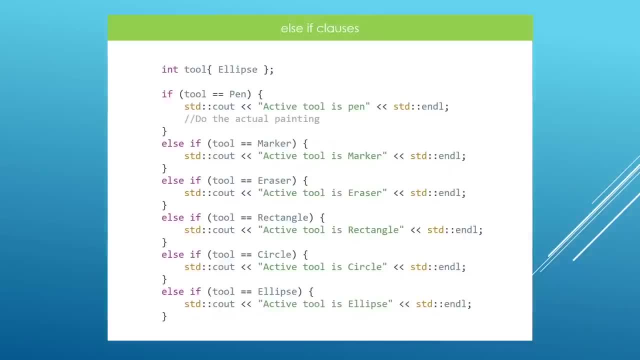 allow you to test for several different conditions. you could do this with a lot of if statements, but that's not going to be really cool. it's going to be ugly and hard to read. this is what you should do. now that you have an idea about this, we're going to head to visual studio code and actually 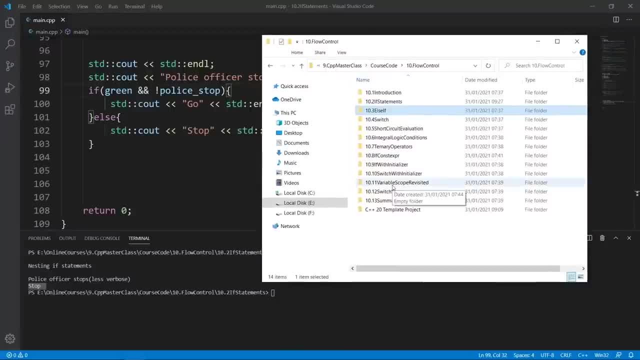 see this in action. here we are in our working directory. we're going to grab our template project pretty quick and we're going to use the else if project here. that's our current project. so we're going to do that and open this up in visual studio code, as we always do. we're going 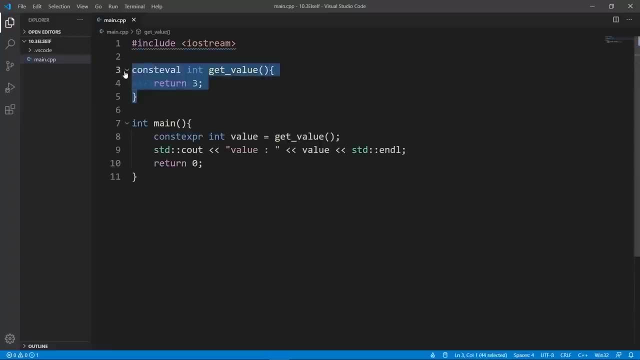 to open this up. we're going to open main cpp and we're going to remove what we don't need. the first thing i am going to do is to put in a set of variables that are going to store our tools, and we can do something like this: we have a variable for pen marker eraser rectangle circle. 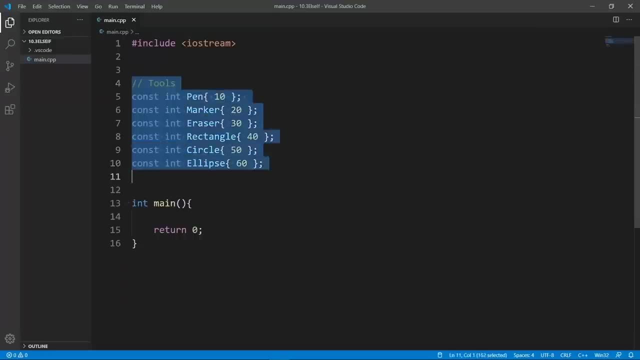 i have to say that this is not the way to go about this. we're going to learn about another way we can do this, but that's going to be later in the course, when we have enough tools to understand this. for now, we're just going to be happy with this, okay. 10 is going to represent the pan. 20 is 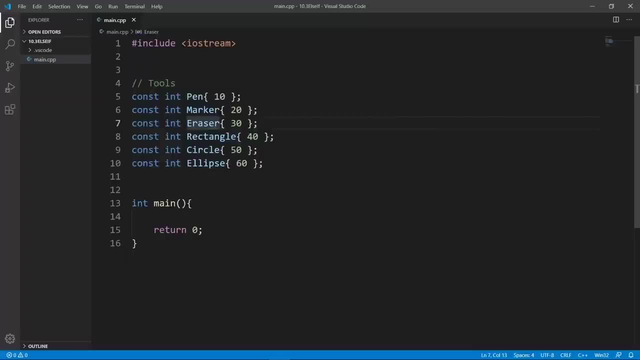 going to represent the marker, 30 is going to represent the eraser, and we can go on until we hit ellipse, which is represented by 60.. now if we go in main and set up a variable and call it tool, for example, and initialize it with whatever tool we think that the user is currently using- for example, we can use circle- 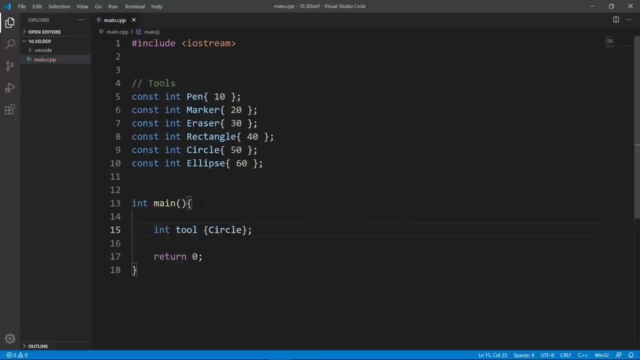 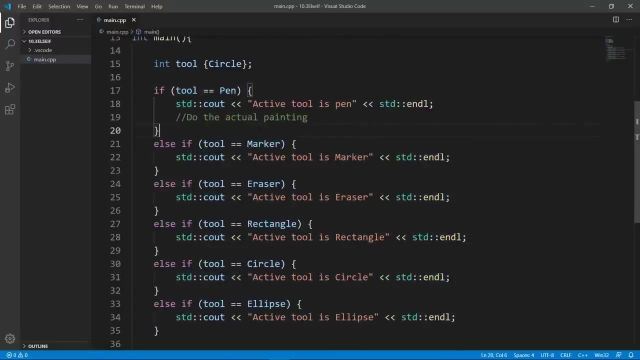 and initialize this. we can set up a chain of if and else if statements to do whatever it is we want to do. when this tool here is selected, okay, we're going to go down and put in our code. i don't want to type all this, so i'm going to put this up here and, if you want, you can copy the code from the. 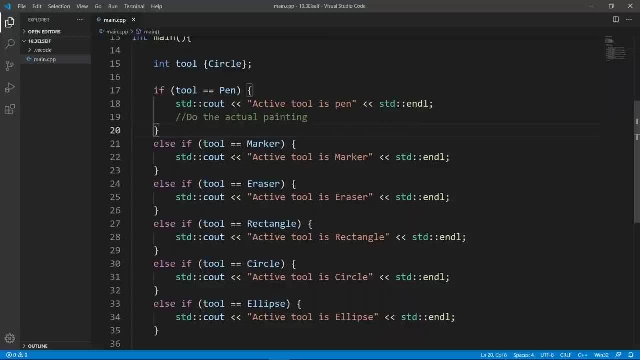 resource section. the code is going to be there. you can copy it and paste it in here and do things with it. okay, we have a chain of if and else. if closes in here- and the first one is going to test and see if the tool is the pan and notice that we are using double equal signs here. this is what you 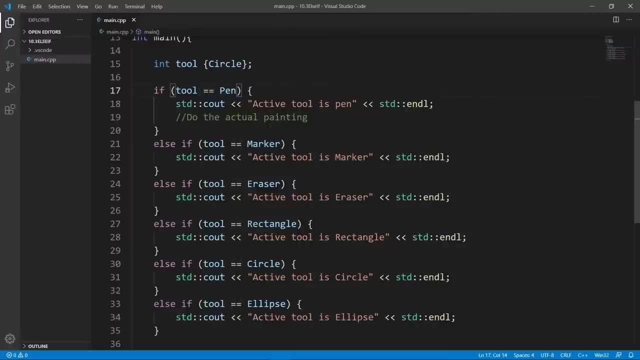 use to test for equality. you don't use one equal sign, you have to use two equal signs. if you use one equal sign, that's going to be an assignment and this is going to always evaluate to true, so you don't want to do that again. to test for equality, you're going to use double equal signs. 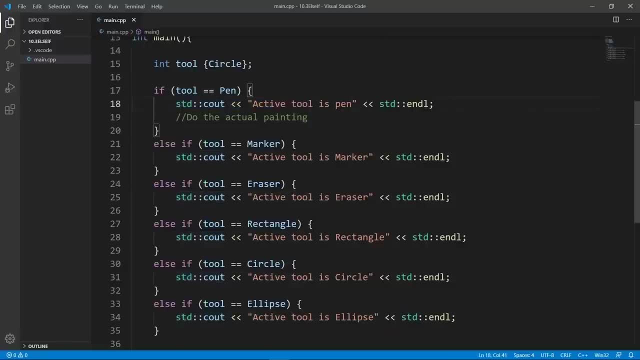 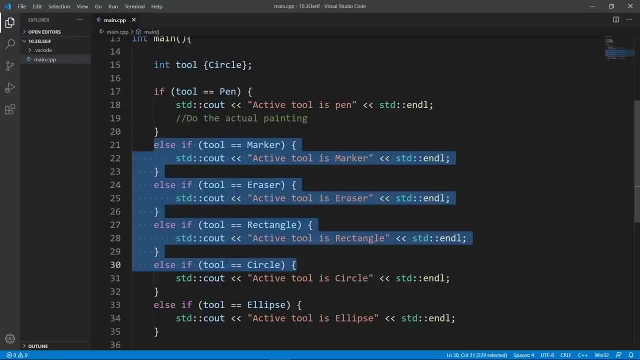 in c plus plus. tool is the pen. we're going to say active tool is banned if the current tool is marker. we're going to say that. so we are basically going to do this for all the tools that our application supports. so what do you think we'll see when we run this? the active tool is circle, so we should print. 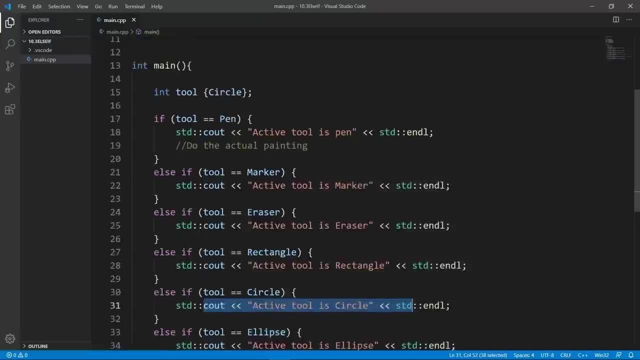 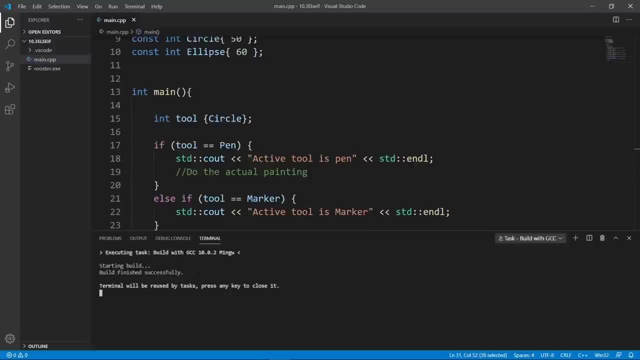 active tool is circle. here let's try this out. we're going to open the terminal so that we can see the output nicely, and we're going to build with gcc and the build is going to go through this. we're going to see active tool is circle. you can go up here and change the tool to rectangle. 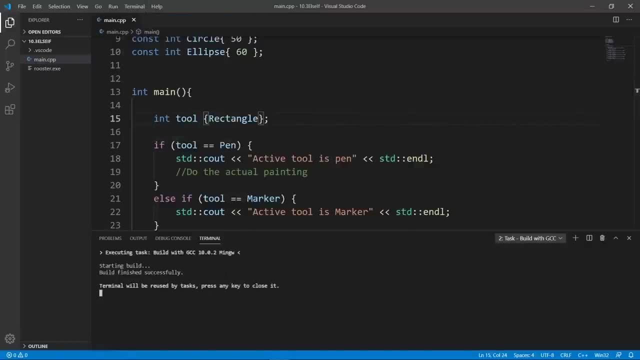 for example, if you build again, you're going to see that the correct block of code is going to be executed. we're going to clear and run rooster. active tool is rectangle. if we try to put in something that doesn't exist, let's say let's put in bird, just to mess with our compiler. here we're. 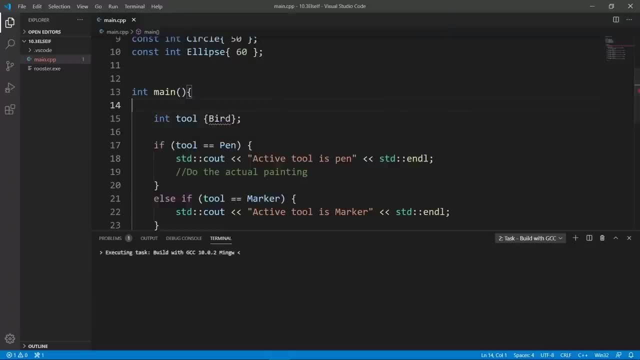 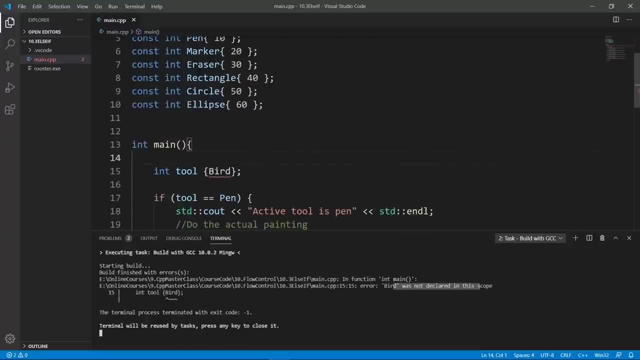 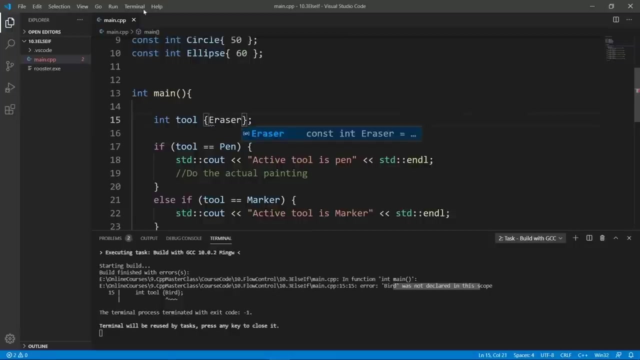 going to get a compiler error because that type is not known by our code here. so we're going to get to declare it in this scope. we don't know what it is. you have to put in whatever thing you have declared beforehand here. so if we put in eraser, for example, we're going to weld with gcc. the build is. 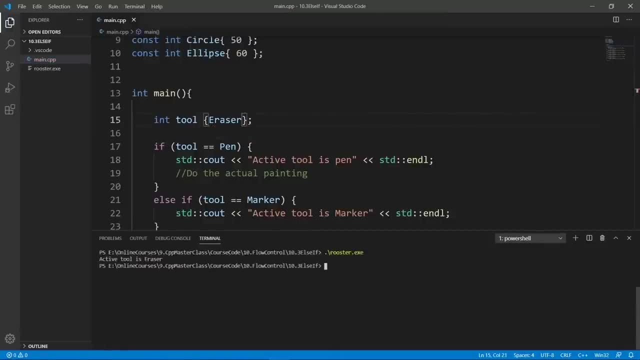 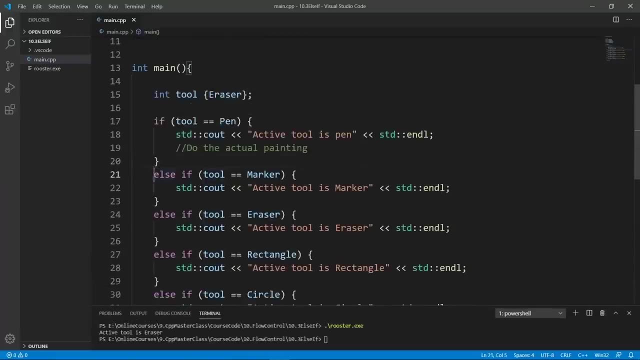 going to go through, going to clear run rooster. the tool is going to be eraser, and this is exactly what we expect. again, the main message in this lecture is that you can use this else if close, if you have several conditions that you want to test for, just like we have here. 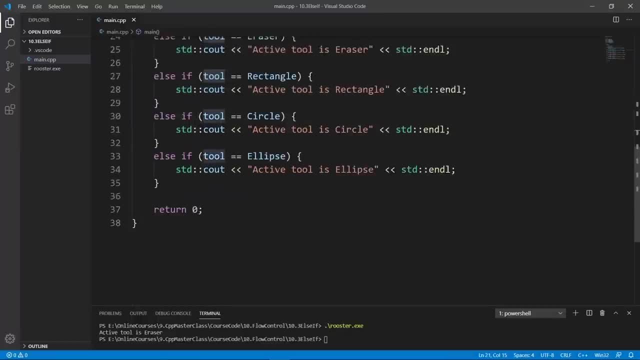 again one of these blocks is going to execute and once we hit the end of this chain of if and else, if closes, we're going to fall here and code after that is going to execute. so let's say: moving on, so that you can really see this here very clear. 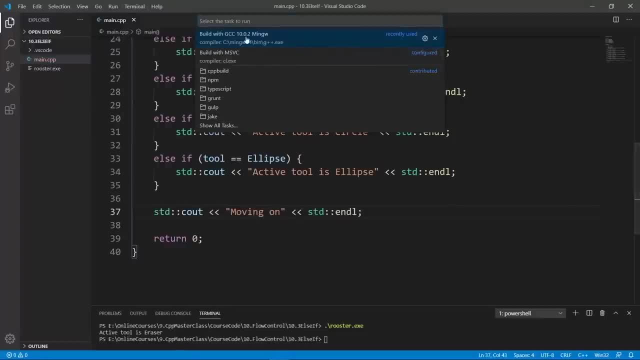 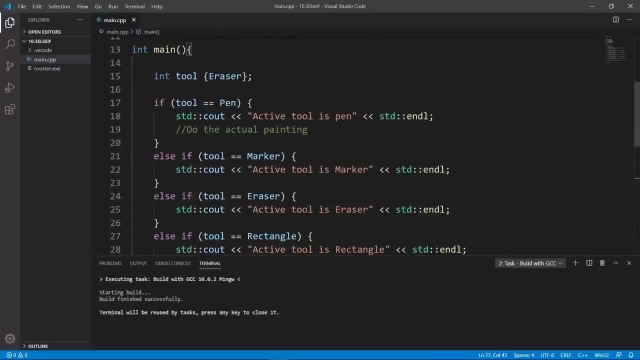 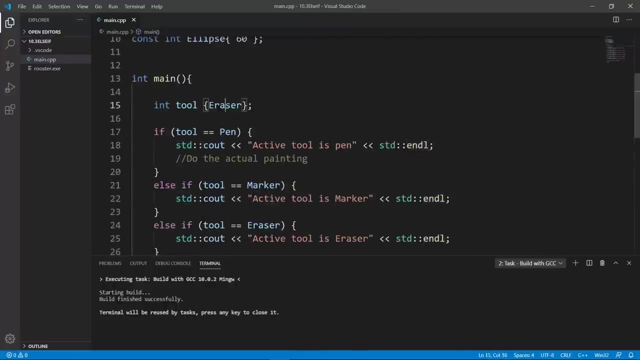 moving on and if we weld this, we're going to see only one block from this whole chain and once one block executes, control is going to go after all this chain and execute whatever is after that. so we're going to say, moving on, after we print that the active tool is eraser here, i think. 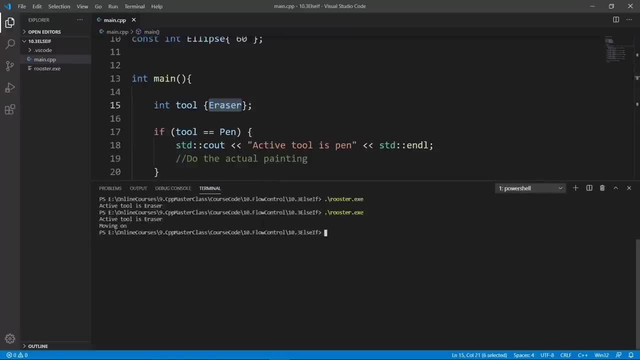 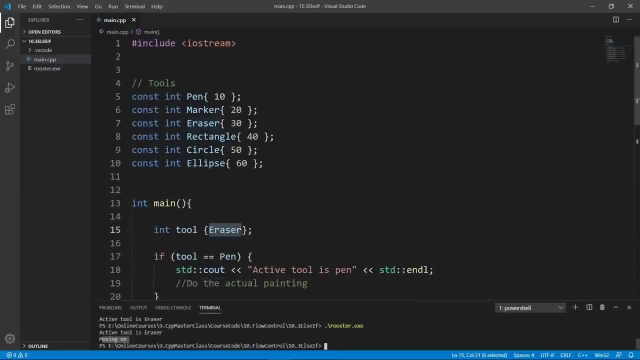 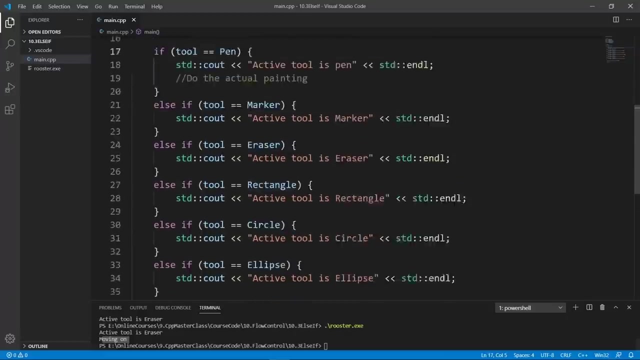 we have both this. so let's try and run this. and you see, active tool is razor and moving on. so after we print the code from the eraser block, we're not going to execute rectangle or a circle or ellipse, it's going to jump at the end of this whole block. this is really what i want to be. 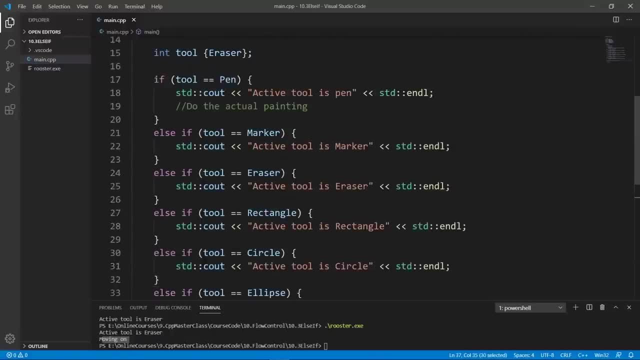 super clear and again make sure you understand the syntax here. the else: if statement is followed by a set of parentheses, and inside the parentheses we have the condition we want to test for. the condition has to evaluate, to boolean, and after that we have the block of code that we want to execute and this is really all you. 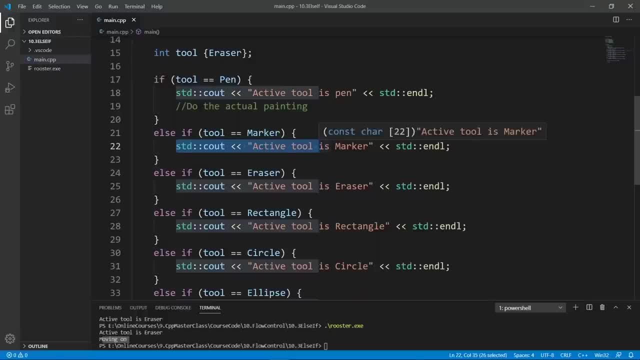 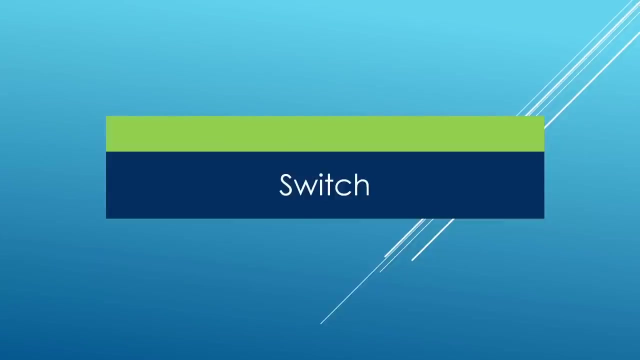 have to do to get this to work to your advantage. we are going to stop here in this lecture. in the next one, we're going to learn about switch. go ahead and finish up here and meet me there. in this lecture, we're going to learn about the switch statement, and this is an alternative way. 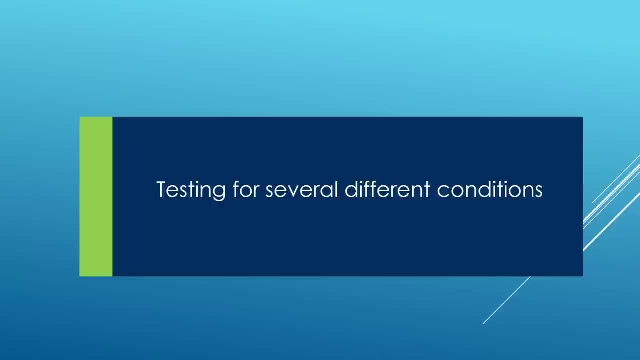 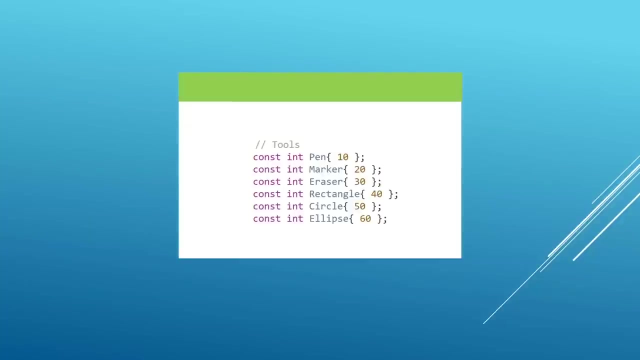 to do what we did with these, else if clauses in the last lecture basically testing for several different conditions, but it's going to be in a much more compact way than what we did in the last lecture. we are going to be using the exact same example we did in the last lecture and we're 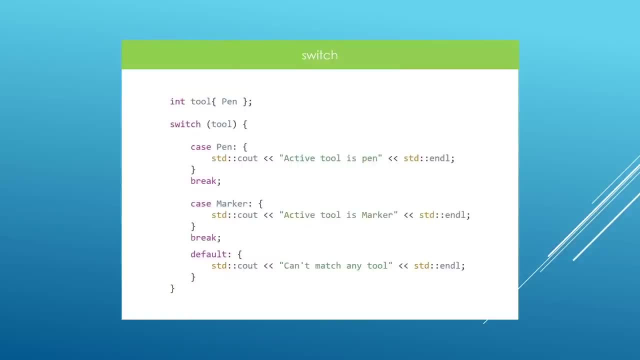 going to look at the switch statement and how it works in c plus plus. and this is how it works. we have our variable which is going to store the current tool, and we're going to say switch inside the parentheses. here we're going to pass the variable. that we're going to be basically. 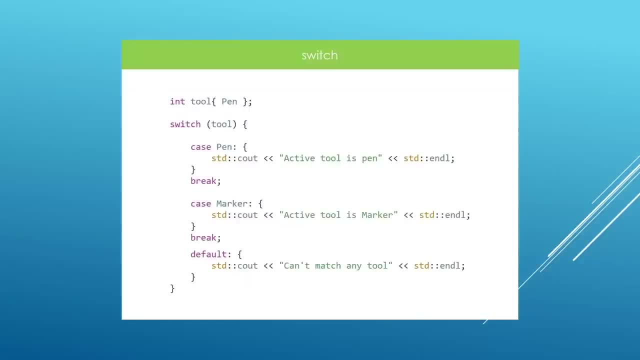 switching on or testing the conditions on and inside the block. we're going to be basically testing for each case. so we're going to say if the current tool is the pan, we're going to say case pan, we're going to put a colon in here and we're going to put the code we want to execute for the case. 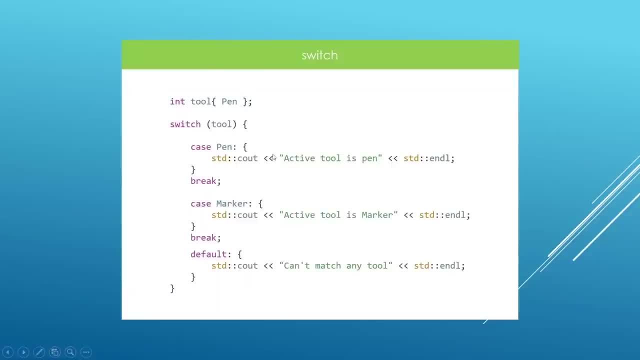 where the current tool is, the pan in these curly braces here. And one thing you should notice from the start is this break statement here. This is a statement that tells C++ that after we successfully execute a block of code, we're going to jump out of this switch statement. 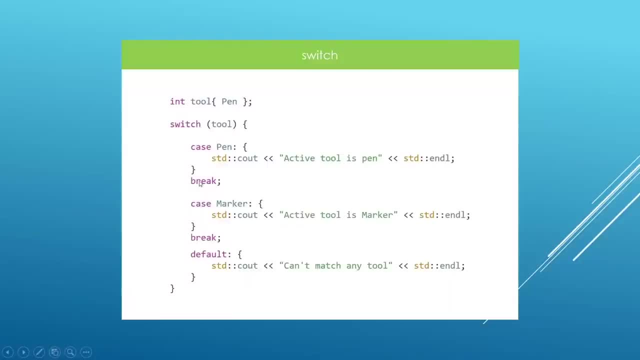 If you omit this break statement, everything after the case that you just executed is going to execute, And that's not probably going to be what you want. If this is not making sense yet, please bear with me. You're going to see it run in Visual Studio Code and you are going to understand. 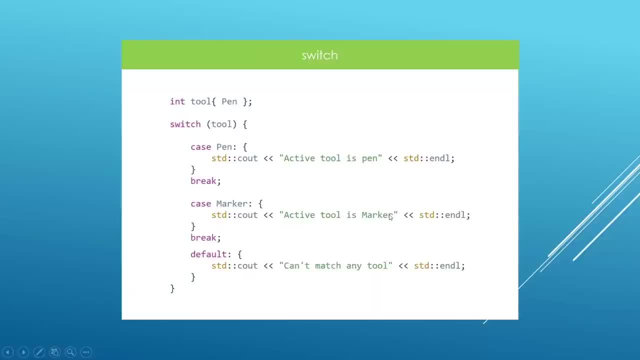 So what you're going to do, you're going to put all the tools you want to test for in separate cases. You see, here we have marker And after that you can put a default case that is going to be matched when nothing has been matched in whatever it is you have tested for in this switch block here. 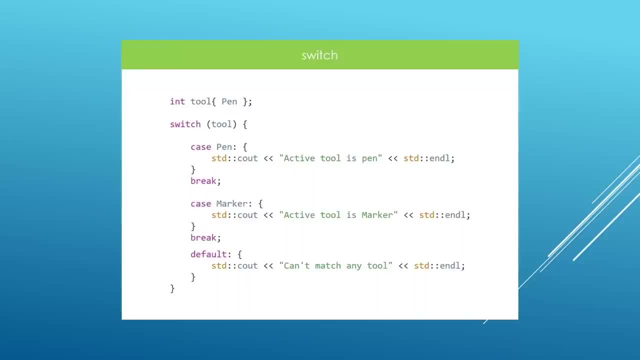 And when we run this piece of code we're going to get exactly the same results that we had in the last lecture, But hopefully you can see that this is much more compact than the series of else- if closes- that we had in the last lecture. 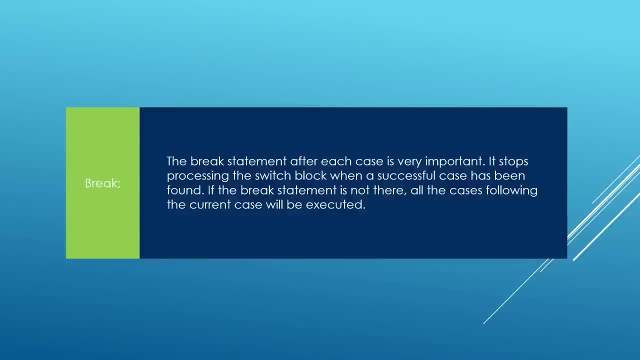 Again, the break statement is really useful. If you don't put it in, C++ is going to be confused And after you hit your successful case, everything after that is going to be executed. So the break statement is basically telling C++. 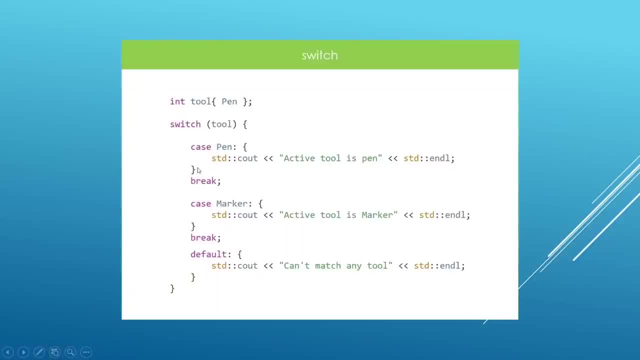 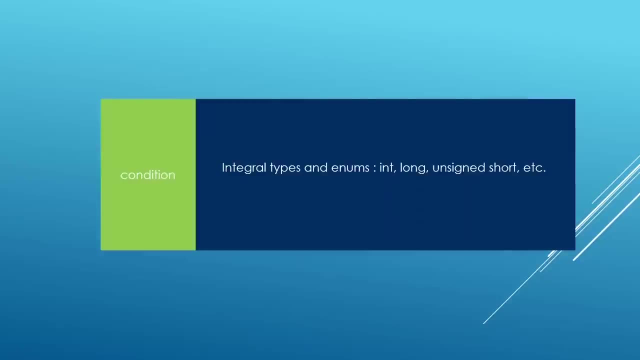 if you hit it after a successful case is executed, jump out of this switch block because you are done. You don't have to do anything else in here. And another thing you should know is that the condition, which is what we have inside this parenthesis here, can only be an integer or an enum. 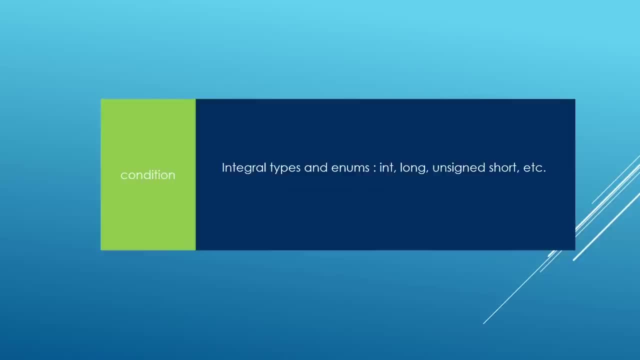 So basically it can be and long unsigned, or car, basically every integral type we have seen before, But it can't be another type such as a string, because that doesn't really make sense. So be sure to keep this in mind now that you have an idea about this switch statement. 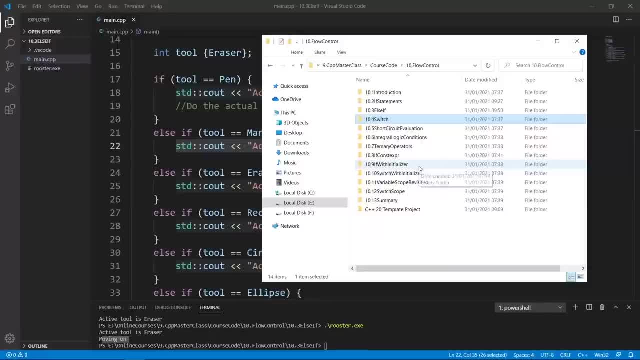 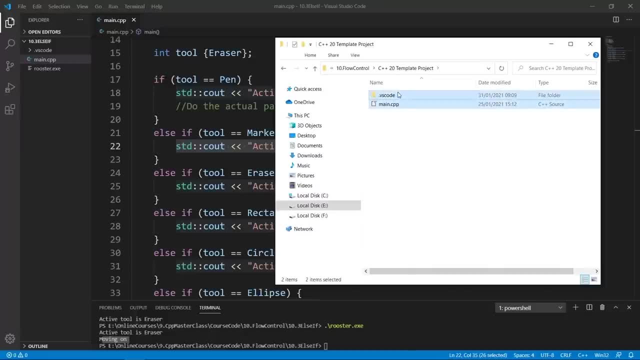 Let's head to Visual Studio code and actually see this in action. here We are in our working folder. The current project is going to be switched, So we're going to grab our template files And we're going to bring that in here. 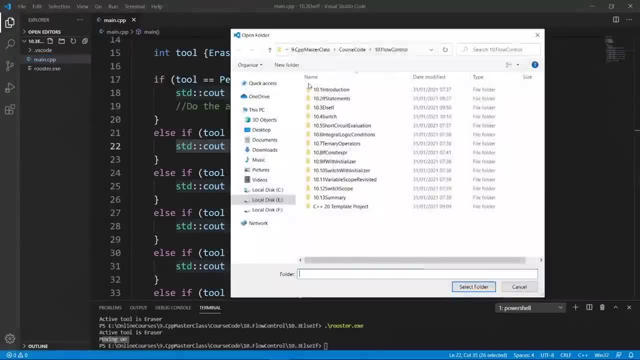 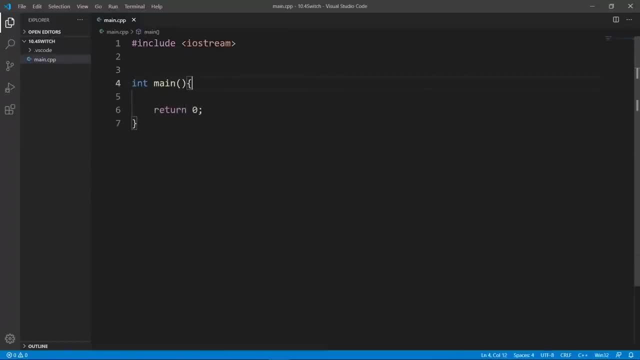 Going to go up a little bit and open this up in Visual Studio code, as we always do, And we're going to open up our main file. We're going to get rid of what we don't need. We going to go outside the main function here and put in our tools, just like in the last lecture. 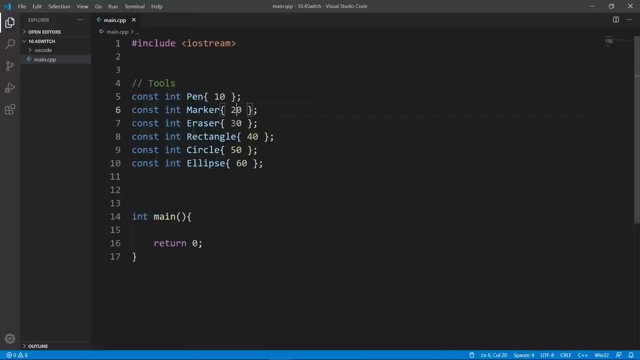 we are using integers. each one is represented by 10, 20, 30 up to 60 and these are the tools we have and i don't think i explained this, but we are flagging them const because we don't want them to be modifiable. we have seen about const earlier in the course. we are going to jump into main and 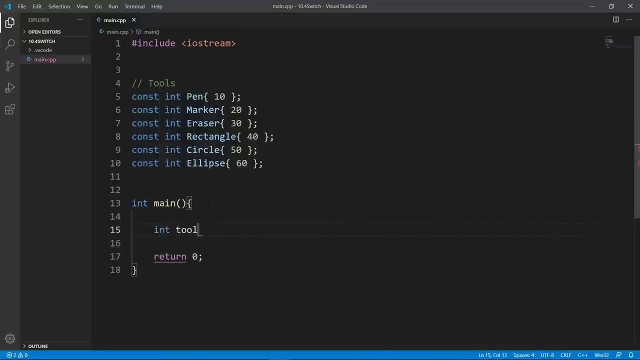 set up our variable. it's going to be ant, and we're going to call it tool and we're going to initialize this whatever tool we want. let's use eraser, why not? and then we're going to put in our switch block. we're going to say switch, and if i type this, you see that visual studio code is going to. 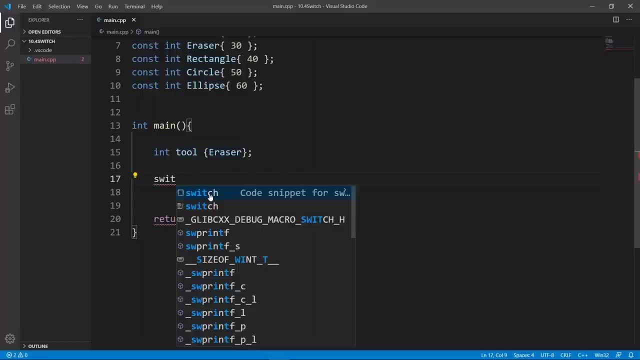 give me intellisense or suggestions on what thing i could do. one cool thing that visual studio code does is give you snippets to really help you type things out. so we can click on this and it is going to auto complete a starter version of our case and we can type in our 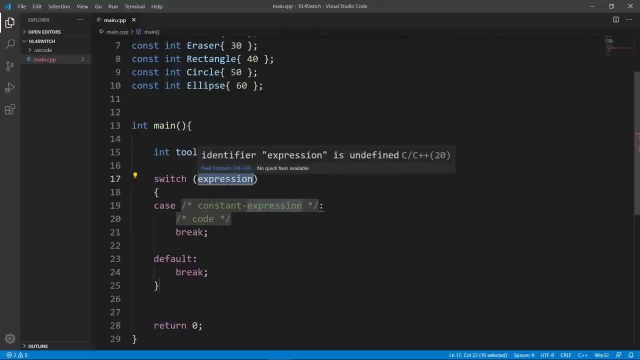 you expression here which is going to be what we're going to be switching over. so we're going to switch over the variable tool here and we can put in our cases. so in our case we're going to start with pan, which is what we have here. so we're going to say case pan, we're going to remove all. 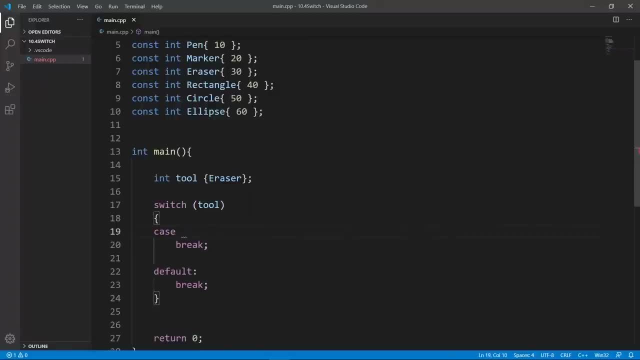 this: uh, let's remove this and say pen. i'm going to put a column and we're going to put a block of code that is going to execute when the current tool is the pen, and we're going to put that in here. let's bring this to the right a little bit and inside the block we can say stdc out. 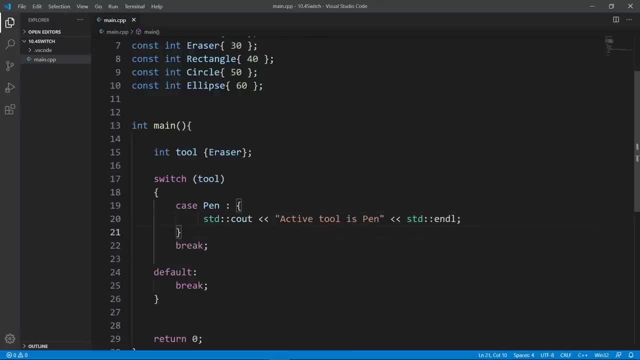 active tool is pan. okay, so after that we're going to put this break statement. if it's not, here we're going to have a problem because when the current tool is the pan and this code here executes, every case after that is going to execute, and that's not what we want. we have to remember to put. 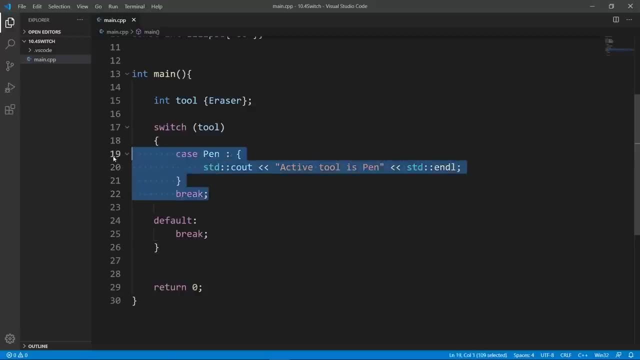 this break statement here. okay, so we're going to put in all our other cases. so we're going to copy this and look at the next one. it's going to be marker, so we can go on the next line and put in marker. we're going to paste this in, we're going to say marker and we're going to say active tool is marker. 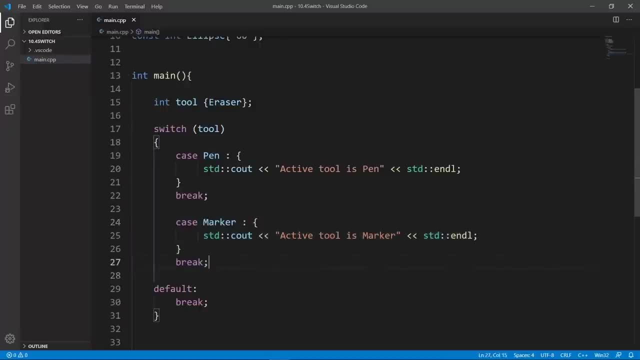 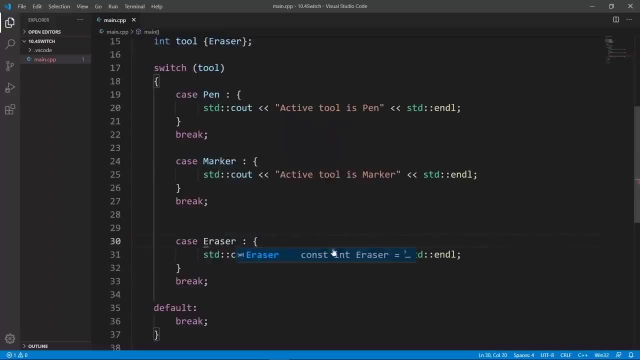 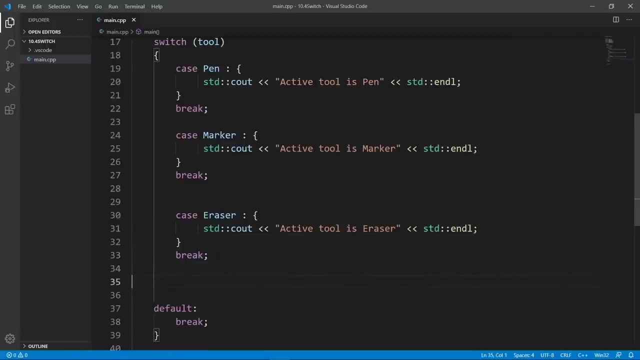 and we can keep doing the same thing. we're going to go down there and paste this in. the next one is going to be eraser, so let's do that. we're going to say eraser and we're going to say current tool is eraser and we're going to go down again. i am doing this live because it really is. 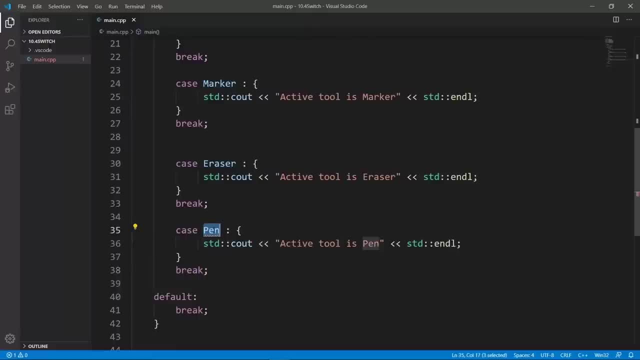 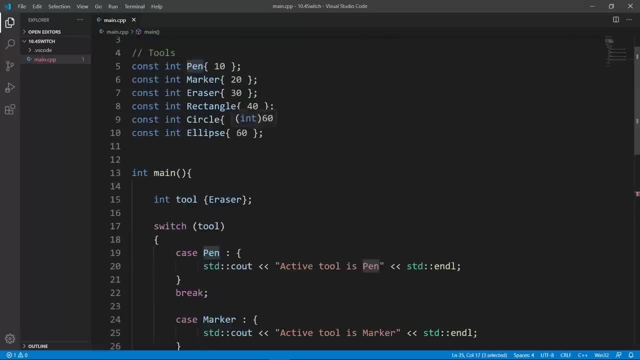 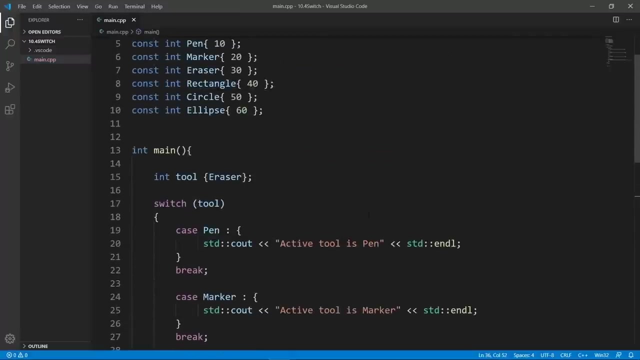 important for you to see me type this, otherwise you may be confused, because this is a slightly confusing construct we have in c plus plus, the next one is rectangle. so we're going to use that and we're going to say current tool is rectangle, the next one is going to be: 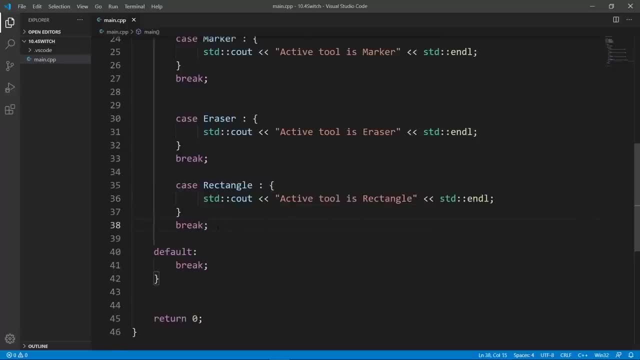 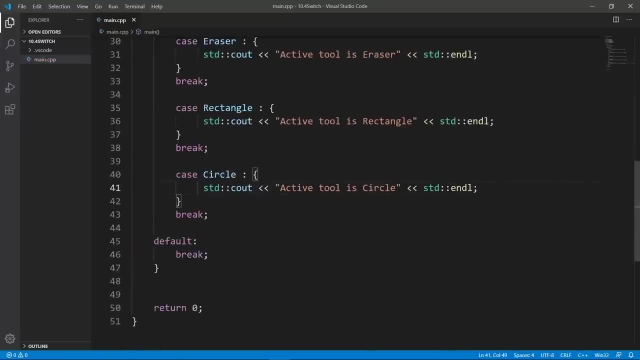 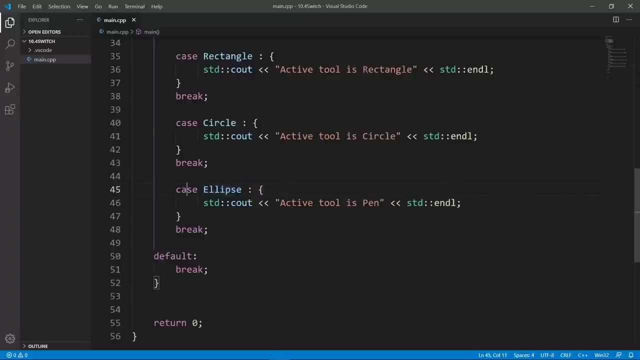 circle and ellipse. so let's do that: we're going to put in circle, we're going to go down and paste this in and bring this back a little bit, and we're going to say circle and we're going to go down and put the next one in, which is going to be ellipse, and after that notice that video studio. 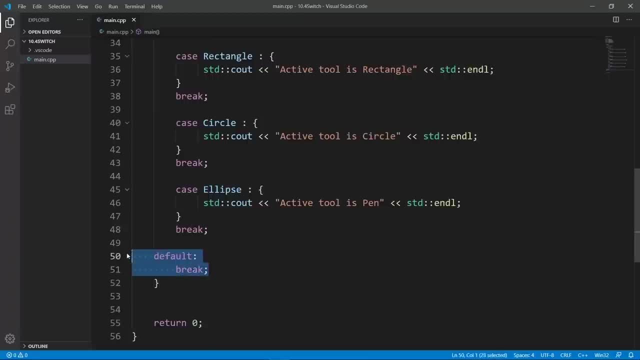 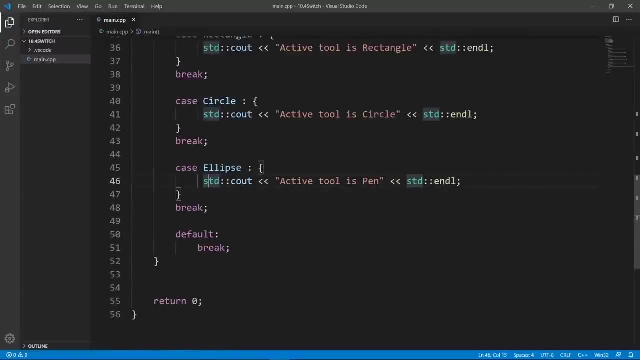 code also inserted a default block, and this is a block that is going to execute when none of the cases here is hit. so this is really important. so you can also add a block of code and say: no match found. okay, so we want to see this print out and we're going to try this out in a minute, okay, after. 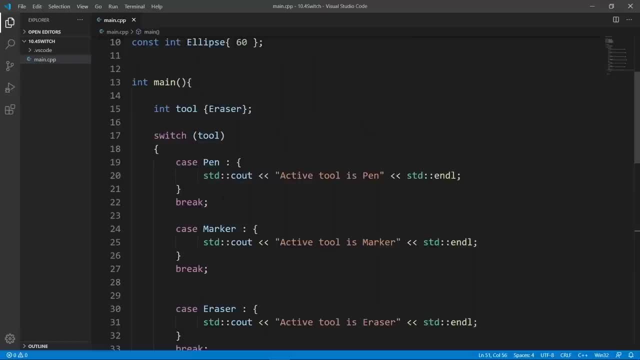 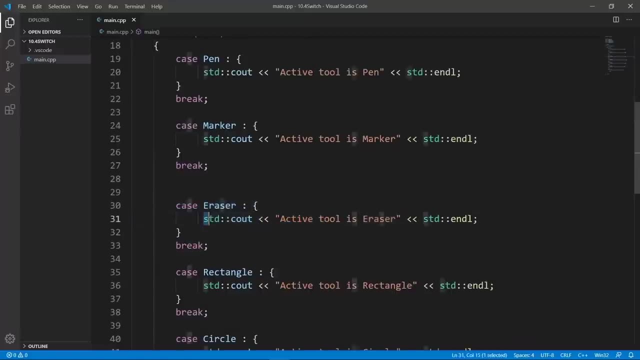 that we should get this to work and do whatever we were doing in the last lecture. so the current tool is going to be eraser, the block here is going to be matched, so code here is going to execute. after that, we're going to meet this break, and what it's really saying is: you have done what you have. 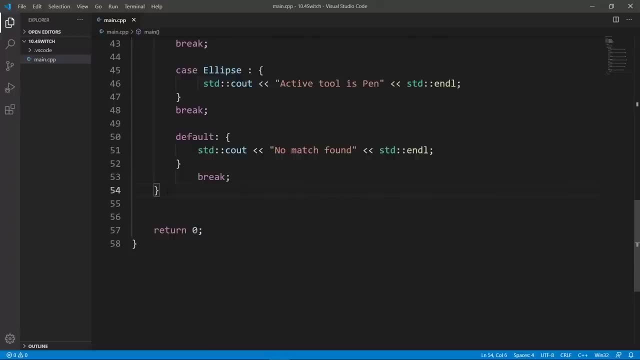 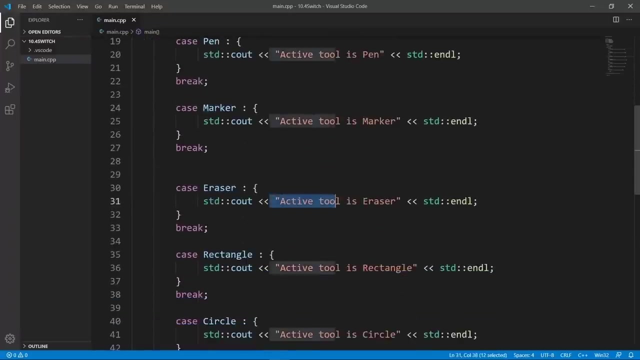 to do: jump out of this switch block here and we're going to go to the end of this switch block and we're going to execute whatever is after that. so just like in the last lecture, we can say: moving on to the program as we have it now, it's going to say active tool is eraser and it's going to print. 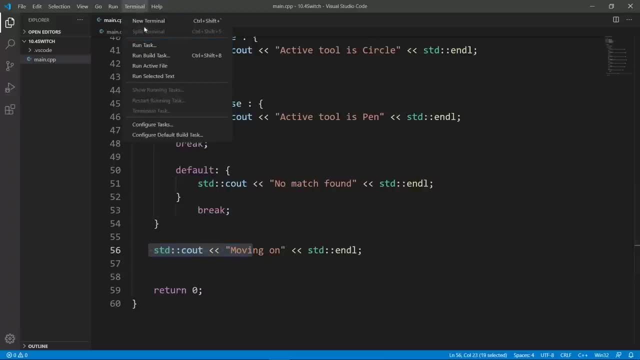 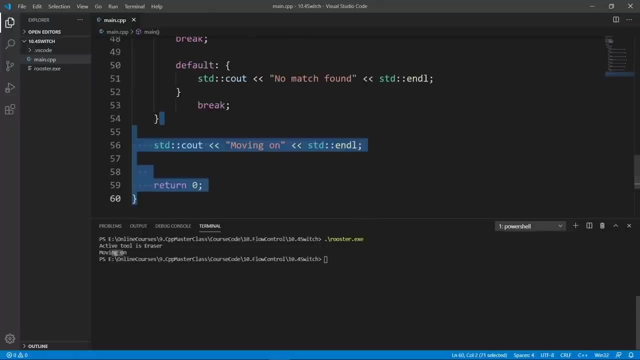 moving on. let's bring up the terminal so that we can really see this, and we're going to build with gcc. the world is going to be good. and if we run rooster- let's clear a bit- we're going to see that active tool is eraser and we are moving on. this is really cool and it is exactly the same thing we had. 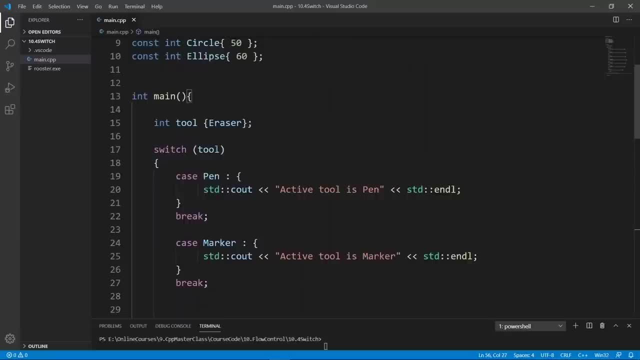 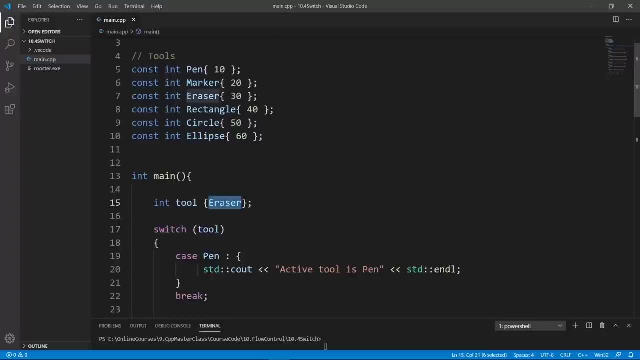 in the last lecture. but now we are using a much cleaner construct which switch provides. okay, we can try to change the tool and see that this really works. we can put in circle- why not? we're going to build with gcc. the world is going to go through, as you see here, and if we run rooster, we're going to see active tool is. 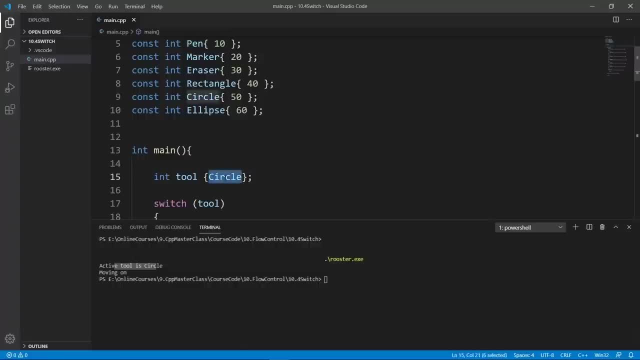 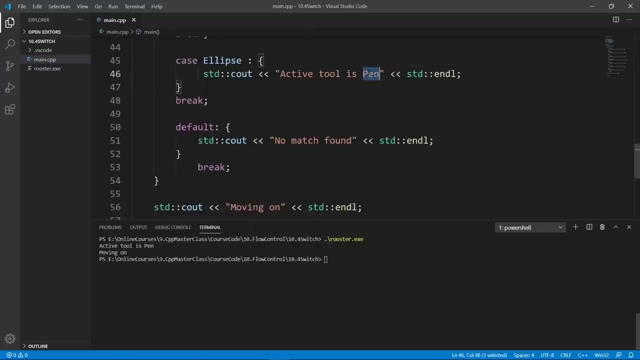 circle. we are moving on. you can try and change this however you want. if we put in ellipse and world again, we're going to world with gcc and if we run, we're going to get active tool is pen and moving on. why is that ellipse? we are saying active tool is pen. we didn't change that, so we. 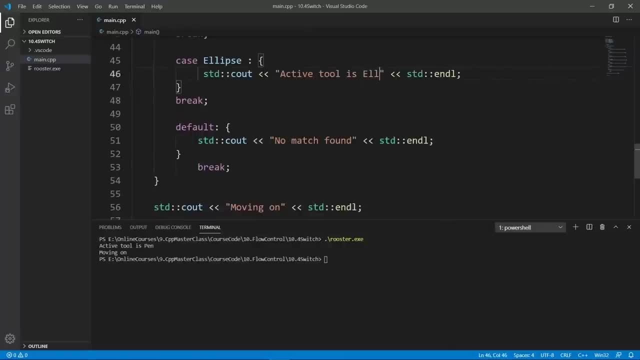 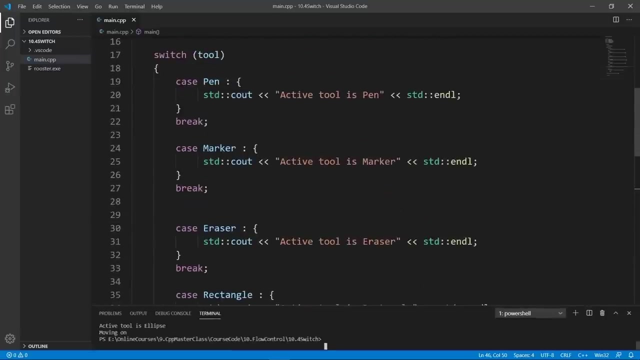 just code a really bad bug here. so let's fix this and we're going to weld again. i'm glad i found this. so we're going to clear and rooster and we're going to see active tool is ellipse and we are moving on, okay. so let's see what could happen if you forgot your brick statement after your case. 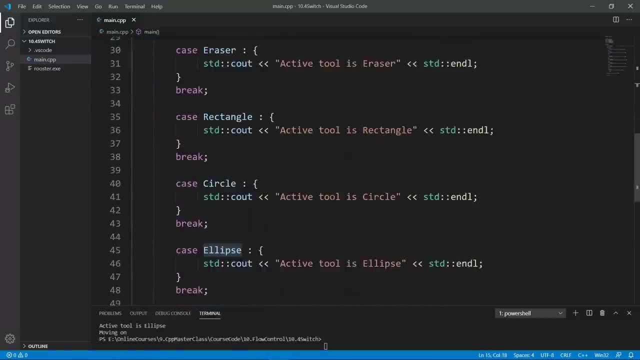 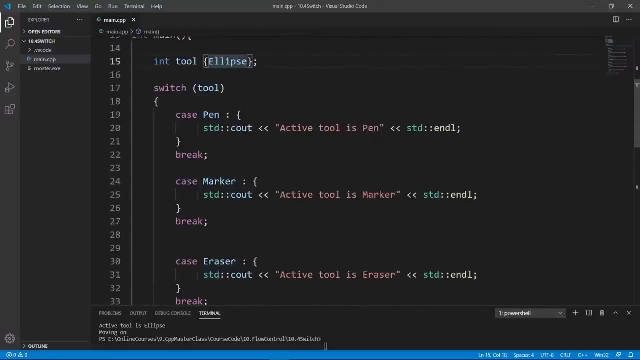 here. so the current tool is ellipse and it is the last thing we have in here, so it's not a good test case. what I am going to do is make the current tool, the pan or the marker. let's use marker. that's going to do, and I am going to remove the break statement here. 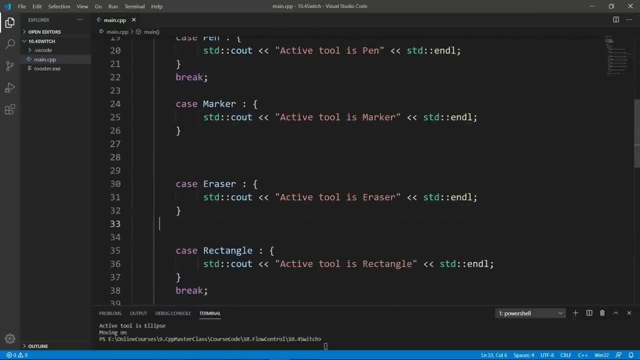 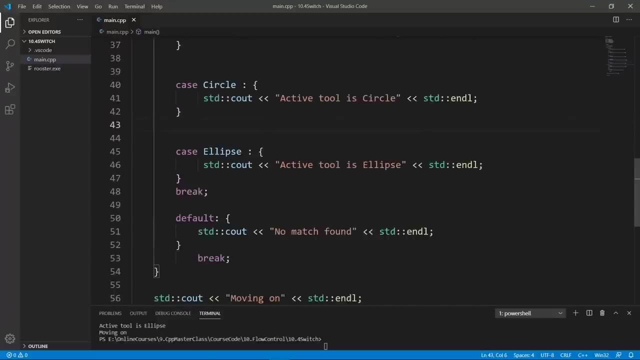 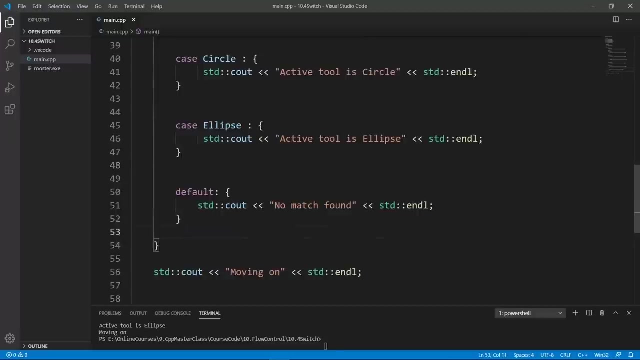 okay so, and I am going to remove all the bread statements we have until we hit the last default case. so we're going to go down and we're even going to remove that for the default case here, and if we're both, we're going to build fine. 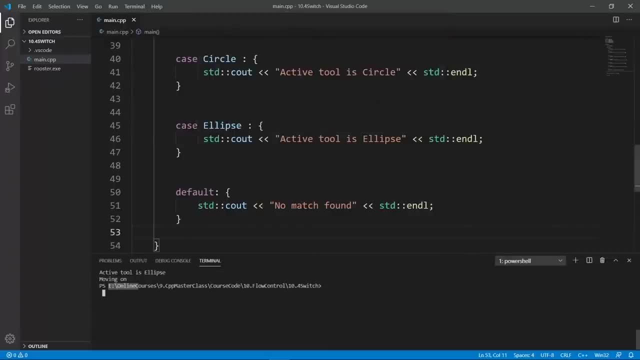 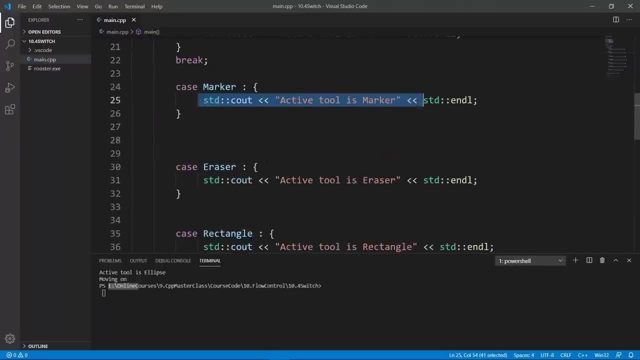 you're going to see that the world was good. but if we run this, try to guess what we're going to get. the current tool is the marker, so we should print marker and hit the end of the switch block and do moving on. but let's do it again. so we're going to hit the end of the switch block and do. 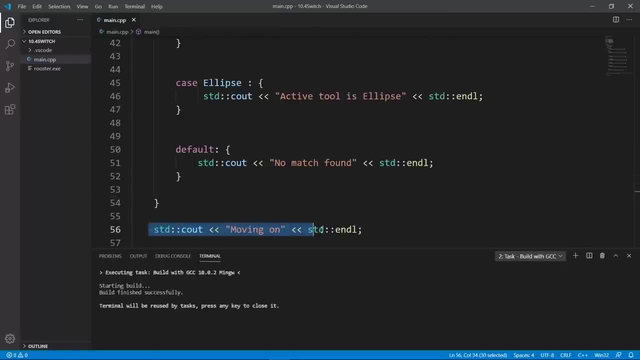 let's see what we get. did we build? let's build again, just to be sure. so we're going to run rooster and notice what happens. active tool is marker. active thought is eraser. active tool is rectangle. we basically print every other case after the marker case is hit and if we try to change this, for example, not. 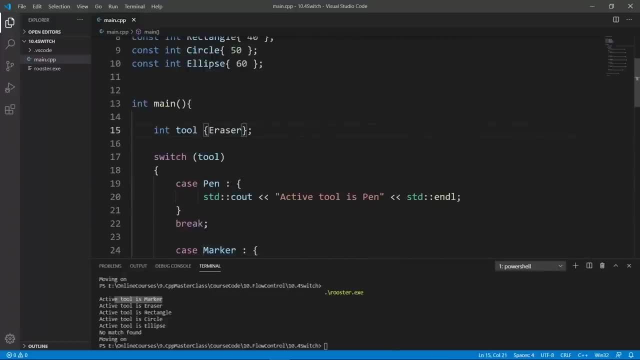 use marker and use eraser. let's change this. you're going to see that we're going to match the eraser case and everything after that is also going to execute, and it is not what you want. so let's clear and run rooster. you're going to see a razor, rectangle, circle, ellipse. 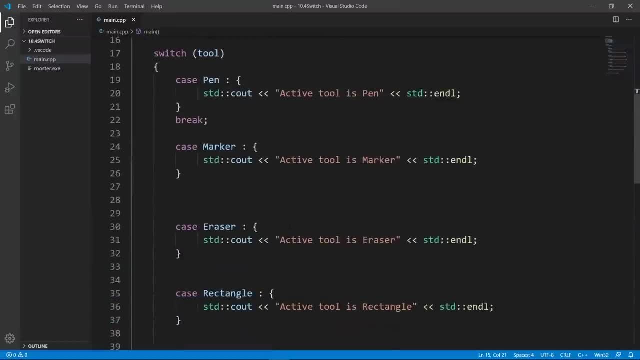 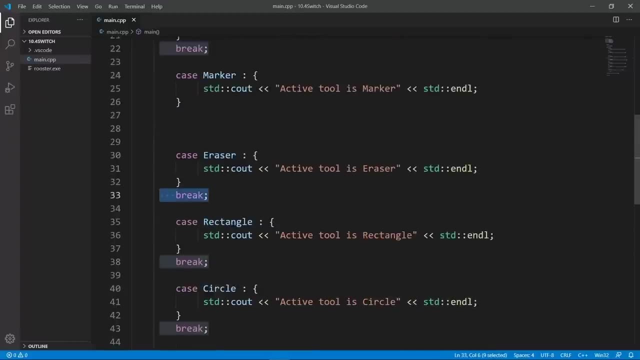 and no match found. so you have ready to remember to put in this break state match. I am going to hit control Z a couple of times and bring those in, and I think this is enough. we have to hit again so that marker also has it and if 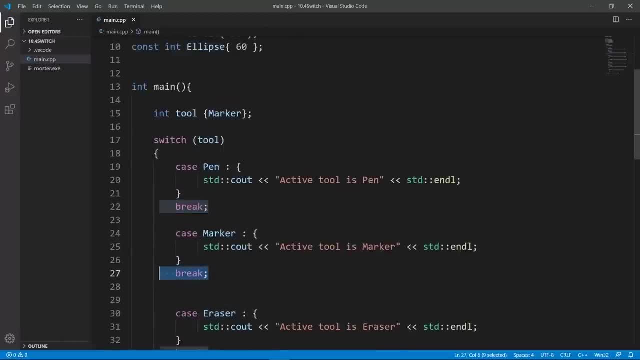 we run now we're going to get what we expect. let's try to use an eraser again and if we build again and click on the eraser and you can see that we've got the message- processingurer ощущation and h SEC dispenser type, where we can see the 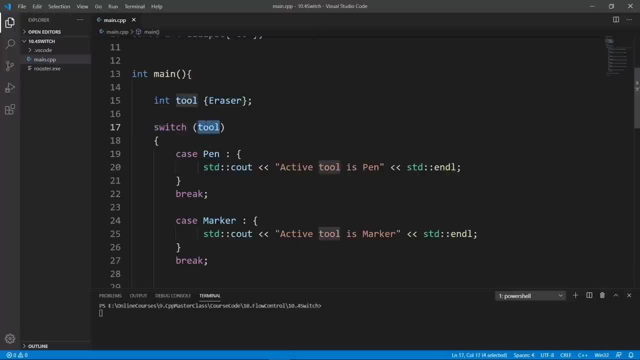 must have left me, guess. lets turn it on then and we close it and it puts in your solution. so we're going to awesomely say, ok, I am going to make sure here that marker is safe. I have our message to read here, our text u in our inbox, in our system our text heading, so it has got to be safe. I am going to keep what I'm wanting. for example, I want to jump into remember: after each case you have to add this book. this is how we work with the standard editor mafias you have to take. 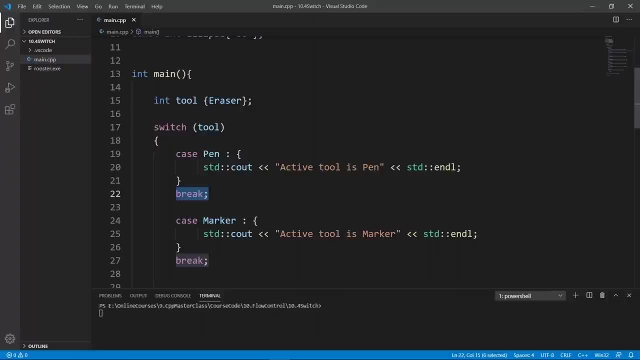 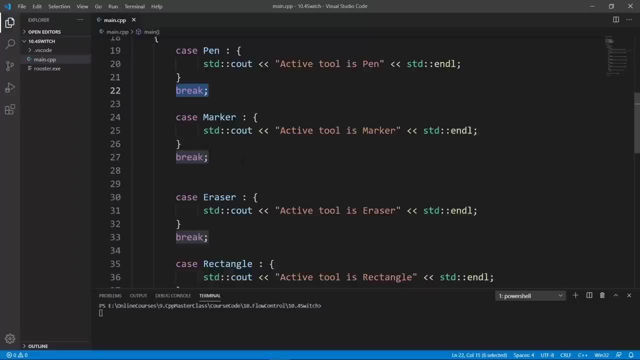 break and remember: after each case you have to add this brick, otherwise you, otherwise everything else after this is going to execute and it is not going to be what you want. before i let you go, i want to show you that you can actually group these case statements. 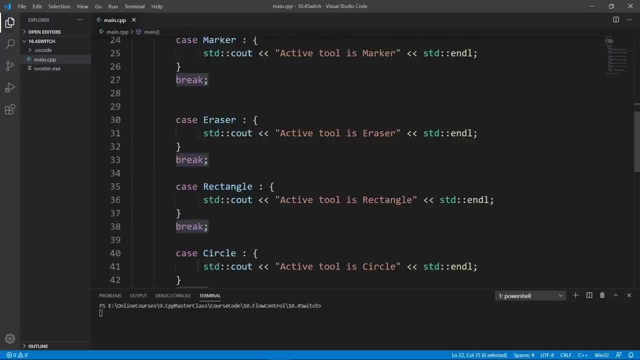 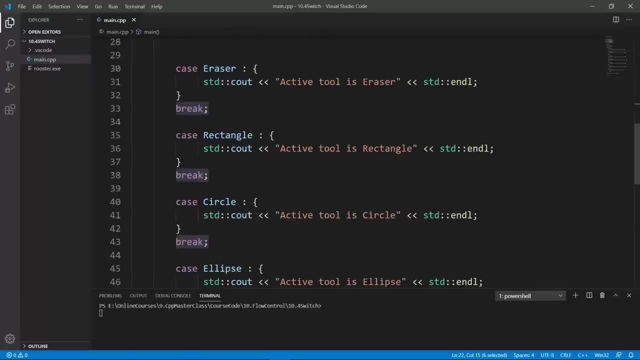 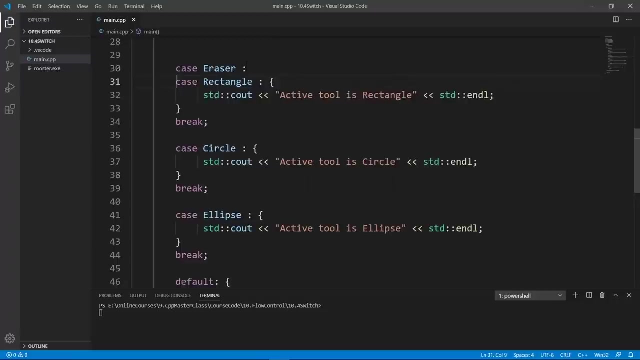 if this is what is making sense for your application. so, for example, for rectangle, circle and ellipse, this can be grouped into the group of shapes so we can actually say case rectangle and put them on different lines, something like this: so let's delete this and say case rectangle, and we're going to delete the other things and say case circle, just like. 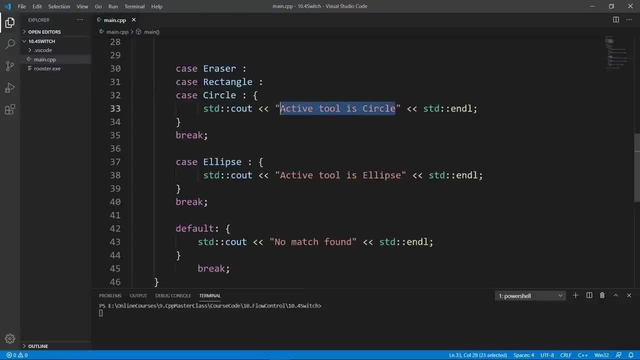 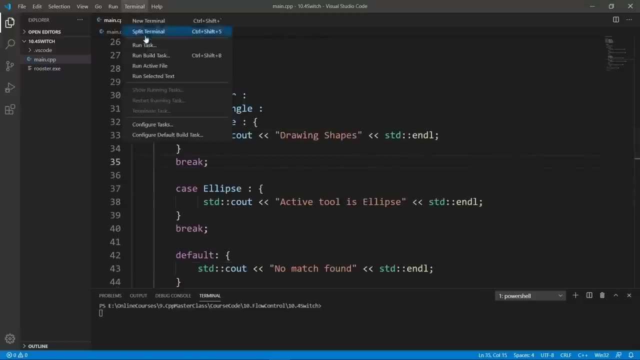 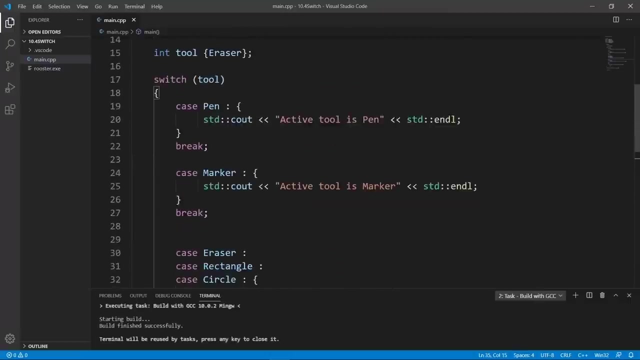 this and we're going to say: drawing shape. i think this syntax is supported in c++. okay, so let's try and world, and we're going to world with gcc and, and the build is going to be good. so if we have eraser, which is what we have in here, we're going 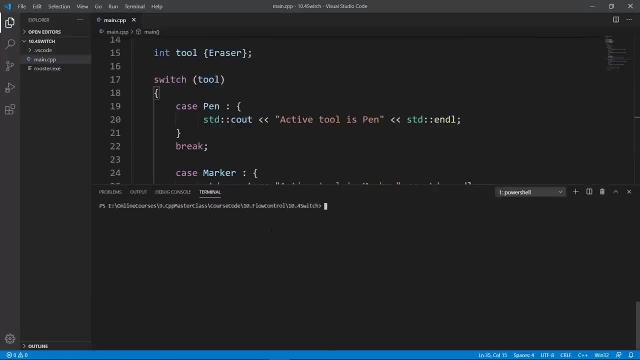 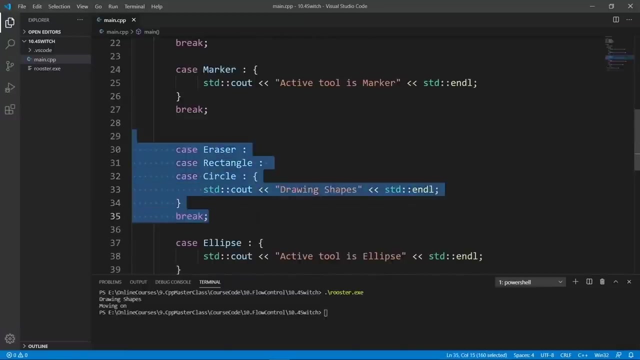 to say drawing shape. let's clear and run rooster. you're going to see drawing shapes moving on. we have grouped different cases and handled them with one block, and this may come in handy in some situations. one thing you should keep in mind is that there are limitations on what you 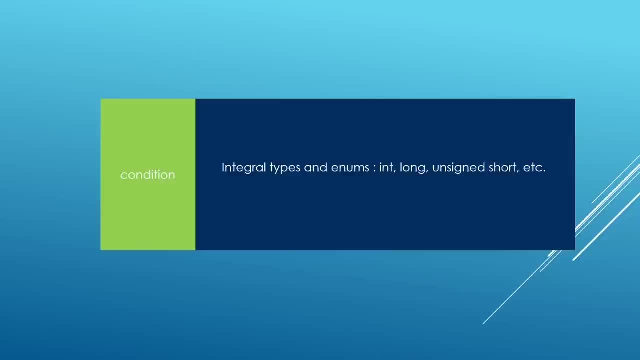 can use as an expression of the case. so if you have a case and you have a case and you have a case and you have an expression of the case and you have a case and you have a case and you have a case, and you have an expression or a condition in your switch statement, and that has to be an integer something. 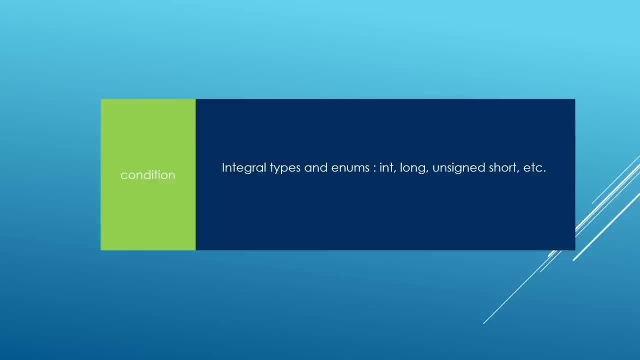 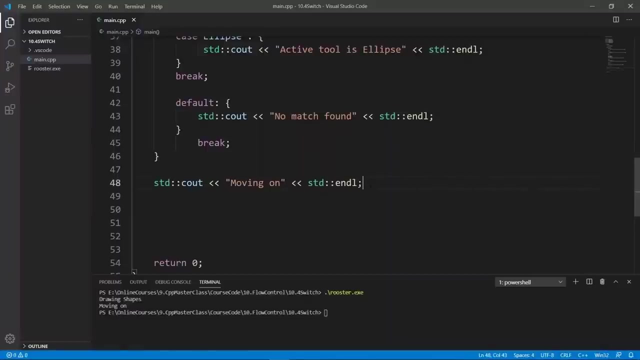 like ant car, unsigned short or things like that. we have seen all of these things, but it can also be an enum. but enum is something we haven't learned about yet. we will learn about it later, when we have enough tools to understand that. but know about this limitation. so if we came in our project, 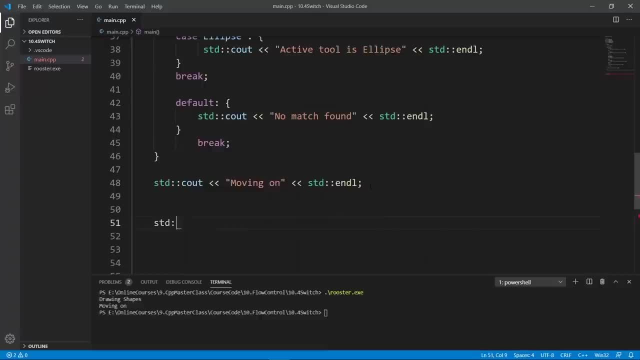 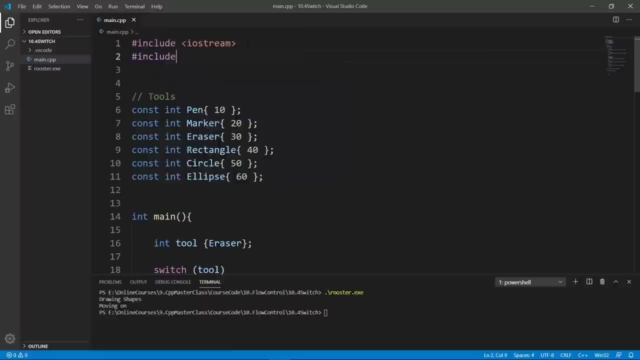 in visual studio code, for example, and say std string name and say, for example: and use this as a switch condition or expression, we have to include string for this to work. so let's go up and include the string library. we're going to do string. and if we go, 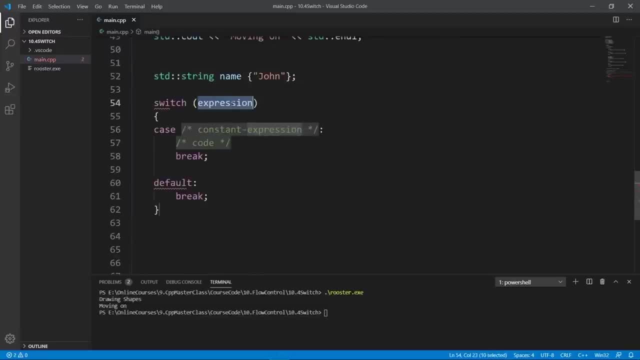 down again and try to do switch and use name as an expression and take out everything we have in here and try to compile this. you see that the compiler is not happy. okay, it's going to say expression must have an integral or enum type. so this is not even going to compile. this is a limitation you have and you have to make sure. 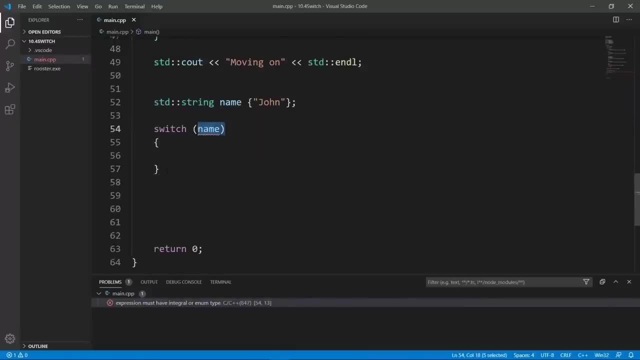 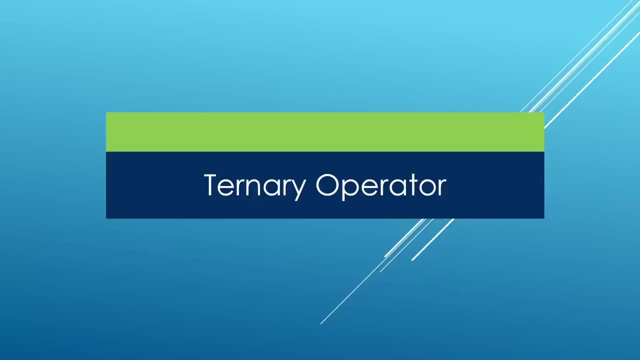 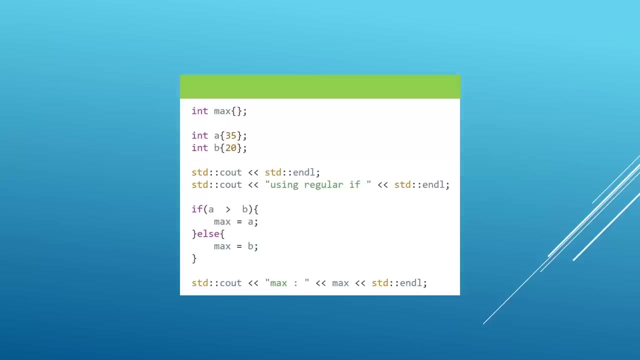 what you pass as a condition here is an integer, something like int or car or other integral types we have learned about in this course. in this lecture we're going to learn about ternary operators, and this is an alternative way to do tests with the if statement. suppose here we have a variable. 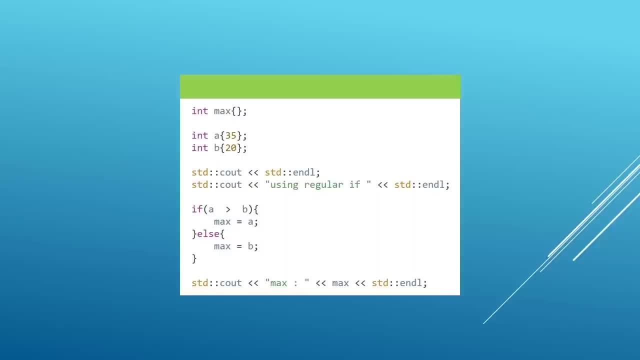 called max. we have two variables called if, and we're going to do a test with the if statement- a and b- and we want to find the maximum between these two things. one easy way we can do this is say: if a is greater than b, we're going to store the maximum in max, else then b is going to be the. 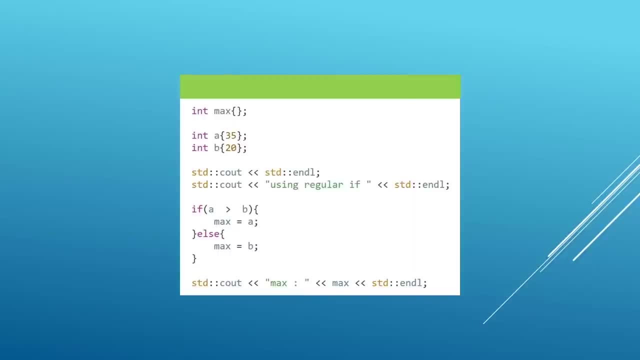 maximum and we're going to store that in our maximum value and we're going to print this out. if we do this, we're going to get whatever is the maximum between a and b to be printed out on the console and this is going to work really well. but we can also use a ternary expression. 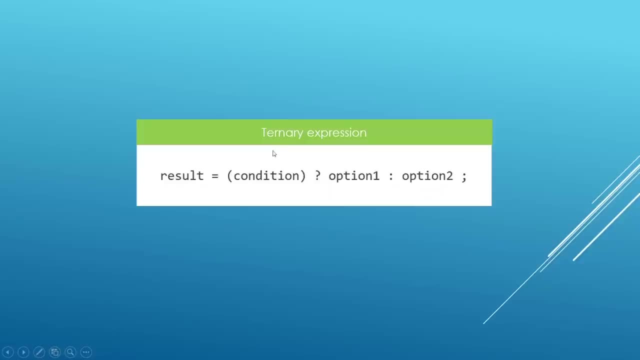 and a expression looks like this and it starts with a pair of parentheses. you're going to put your condition inside the parentheses, you're going to follow that with a question mark, you're going to put your option 1 and after that you're going to put a column and option 2, and because this is a state matching C++. 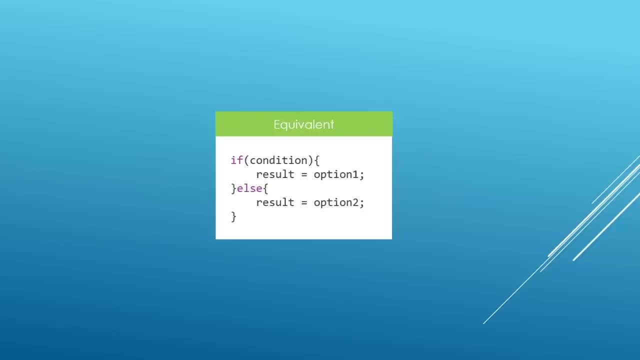 we're going to end this with a semicolon. here is an equivalent version of that using F, as we have been doing all along. so we say: if condition result equals option 1, if condition is false, result is going to be equal to option 2, and this: 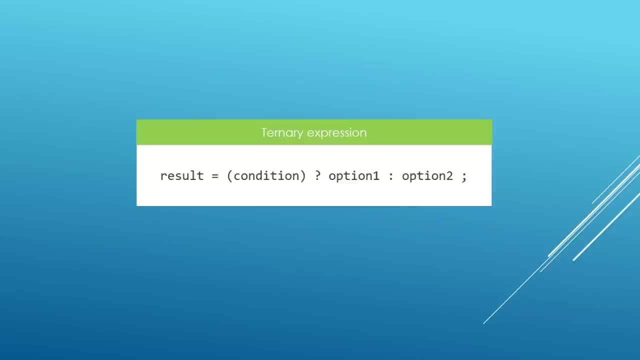 is exactly the same thing we are doing with our Turner expression here. if the condition is true, we're going to take option 1 and assign that to result. if it's false, we're going to take option 2 and assign that to result. so this is. 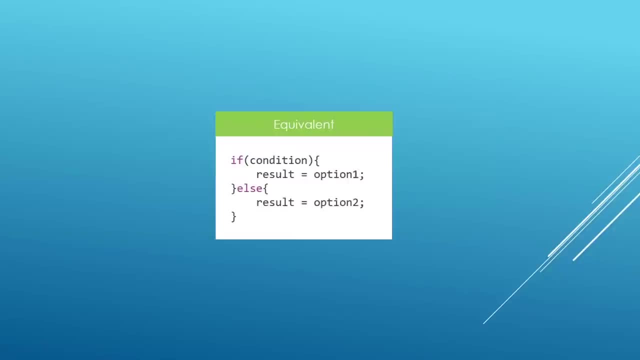 really a synthetic sugar or a shorthand for this thing here, and it's going to make your code shorter and you're going to see this all over the place in a C++ code out there, so you really need to be familiar with this, okay, so here is our example of 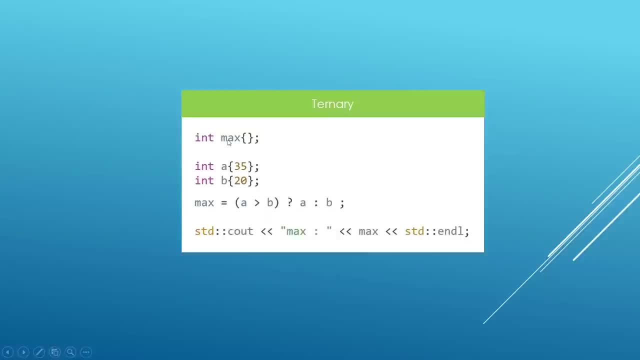 computing the maximum. you see that we have the same variables, max a and B, but we have a one-liner that is going to store the maximum and max and we can print this out and hopefully you can see that this is shorter and better than this. okay, one other thing you should know is that option 1 and option 2 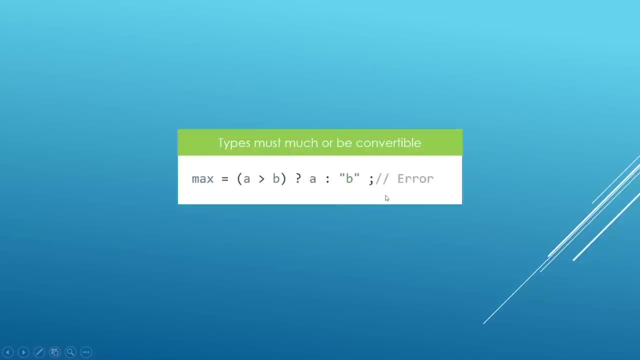 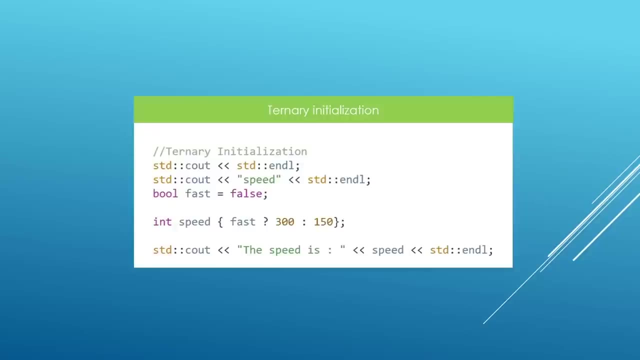 should be of the same type, or at least the types must be convertible, and if that fails you're going to get a compiler error. we can also do ternary initialization. here we have a boolean called fast. we initialize this to false. we can use this to initialize our speed variable. here we are basically saying: if 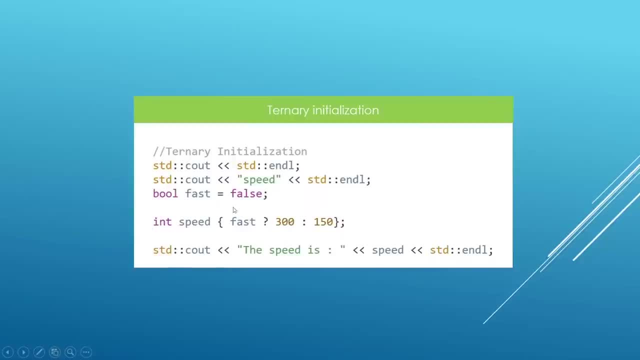 fast, initialize this with 300. if not, fast, initialize this with 150 and we are going to print the speed here and this is going to work. and here you see that I lied a little bit in my explanation to make it really obvious what we had in our ternary expression. you don't have to always wrap your 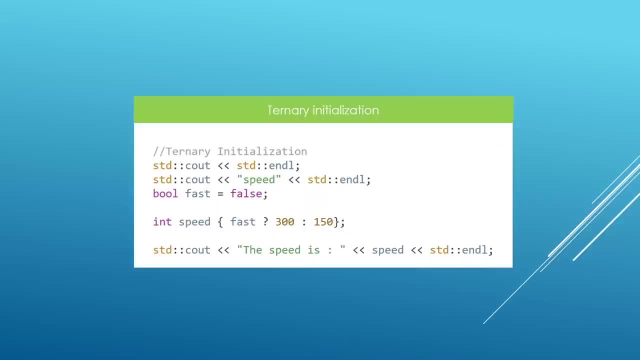 condition in parenthesis, but it makes the code much cleaner. okay, now that you have an idea about this things, it's time we headed to Visual Studio code and actually tried this, and so for ourselves: okay, here we are in our working folder. okay, here we are in our working folder. okay, here we are in our working folder. 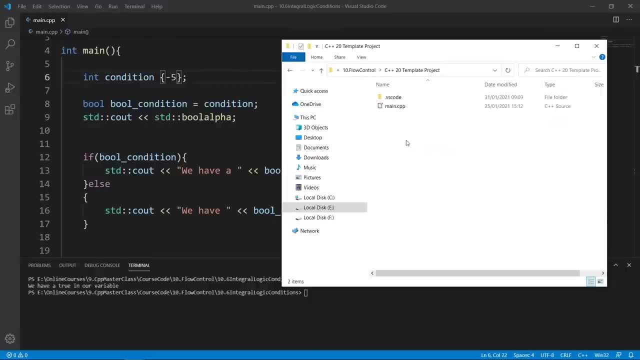 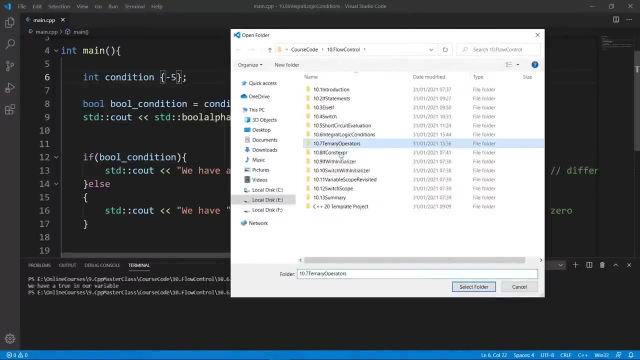 the current project is ternary operators. we're going to grab our template files and put those where they belong- it is in this lecture here on ternary operators- and we're going to open this up in Visual Studio code, as we always do. we're going to open this and we're going to open main CPP and take out whatever we 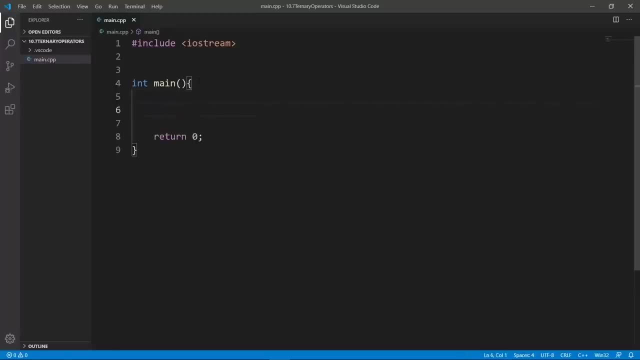 don't need. we are going to go down and put in our test code. we basically have a few variables. let's kill these spaces so that our code is not clattered here, and we're going to print our maximum and we're going to be using a regular. if we have three variables- max a and B, we are. 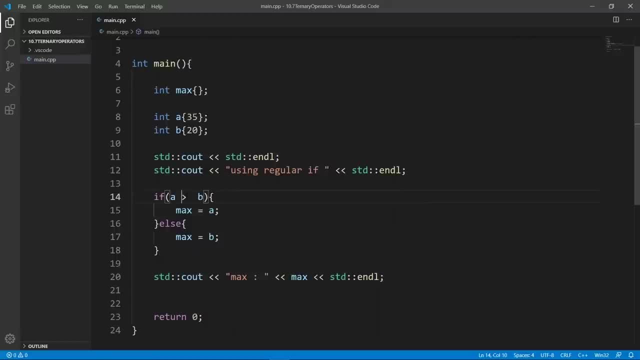 saying, if a is greater than B, we're going to store the maximum in max. otherwise, we're going to store B in max and this is going to allow us to print whatever is the maximum between 35 and 20. if we build this, let's bring up a. 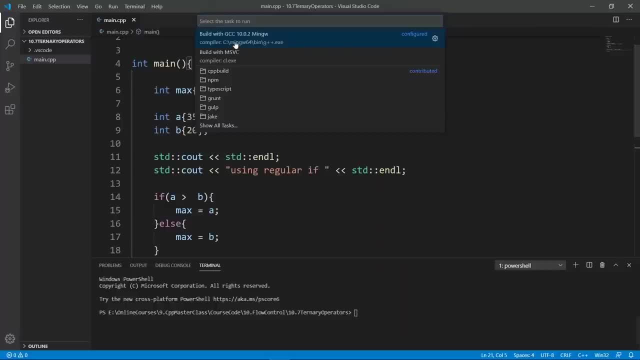 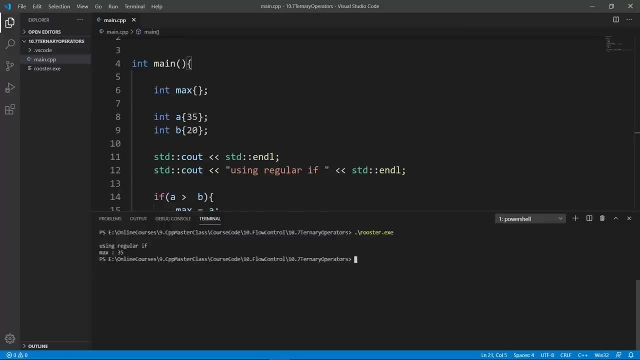 terminal and to build with gcc, as we always do. let's bring this up a little bit and we're going to clear and run rooster. we're going to see that the maximum is 35. if we put our maximum in a beam, we're going to get the maximum steel. so we're going to run the task to build with gcc. 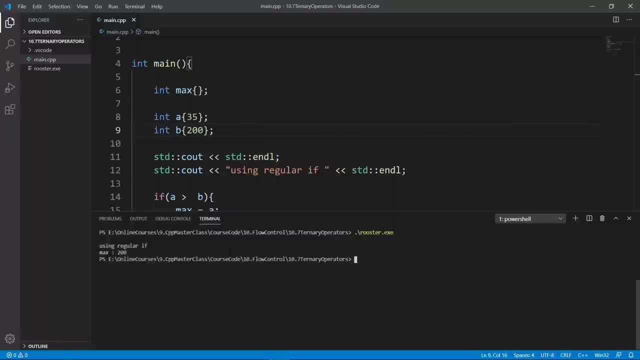 and we're going to run this clear rooster max is 200, so we're going to get the maximum, regardless of where it is stored in, a or b. this is how our code works, but we can use ternary operators to do the same thing. so what we're going to do here, we're going to comment out our if. 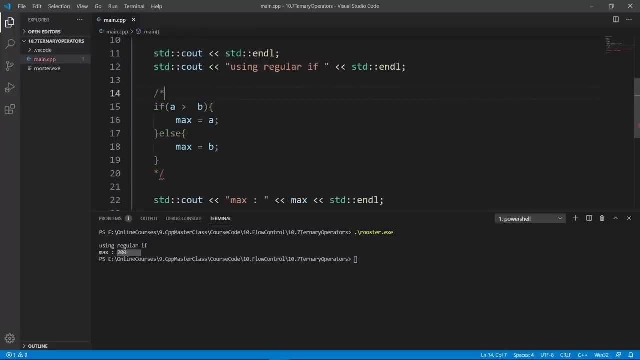 statement and use a ternary version. so what we're going to do? we're going to say result equals and we're going to say a greater than b. we're going to put a question mark to signal the start of our two options. option one is going to be a, because if a is greater than b, then a is going to be the maximum. 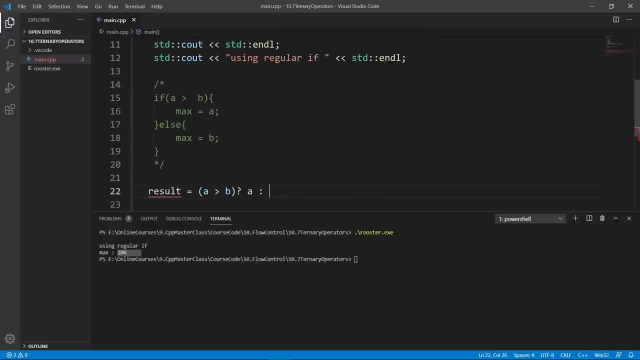 so we're going to grab a here, and if a is not greater than b, then b must be the maximum. so we're going to put that as a second option here. this is what we mean with this statement, and we don't have a variable called result. that's why we have a problem here. we're going to put our 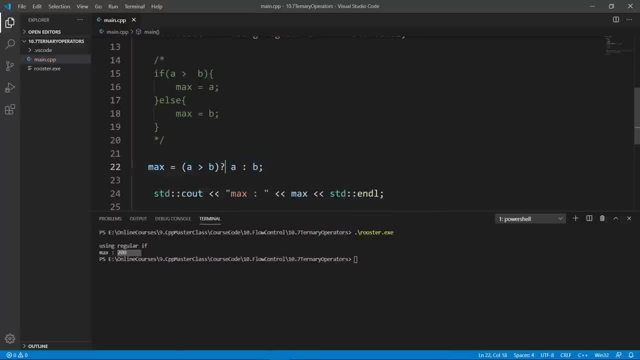 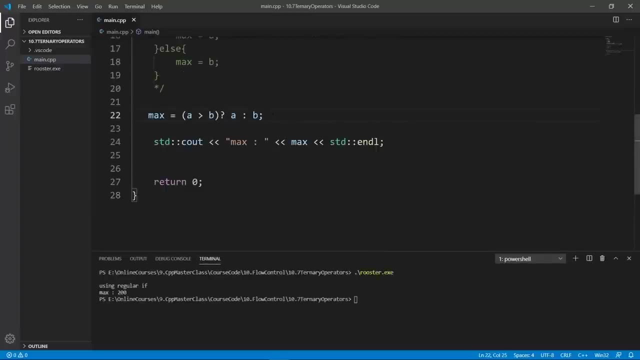 result in max and this should solve this problem. you see, the squiggly lines go away and we can build this and we're going to get exactly the same result. so this is our ternary operator. if we build this, it is going to go through, and if we run this, we're going to get. 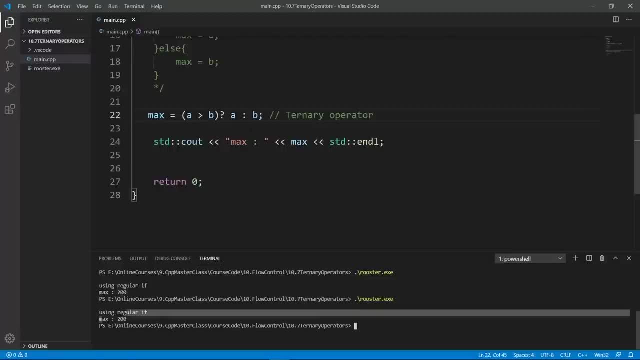 exactly the same result. max is 200, and it is what we expect. okay, so take some time and really make yourself familiar with this syntax. it is really nothing complicated. you just have to make sure your brain is aware of something like this and you're going to recognize it every one. 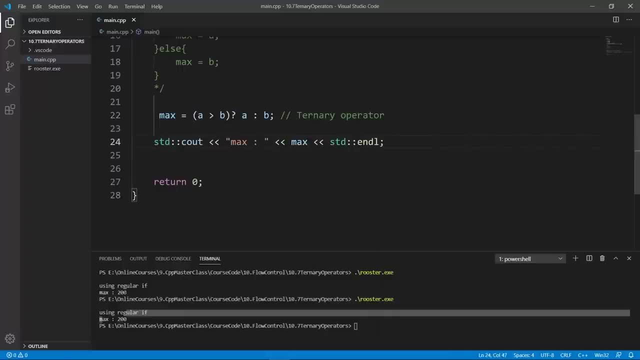 where you see it in code out there. okay, we have mentioned that you can't pass types that are not compatible and the requirement is that a and b be of the same type, or at least types you can do conversions between. so, for example, if we try to do something like pass a hello in here, we can't. 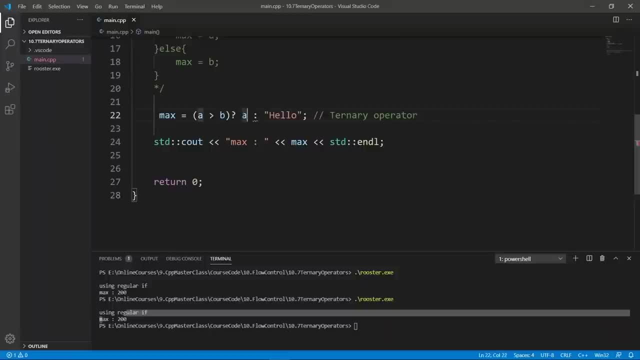 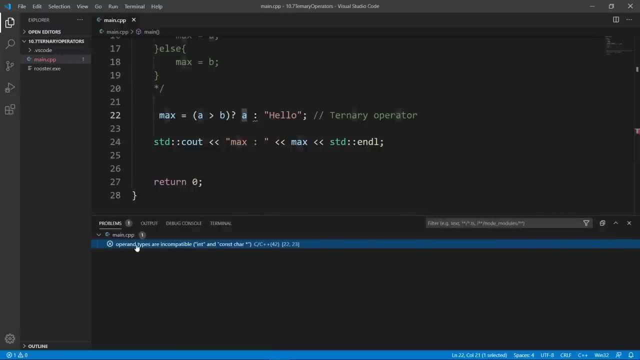 really turn a strength into a, an integer, and this is going to give us a compiler error. and let's look at the error we see from visual studio code: operand types are incompatible and and the const core are not compatible and they have to be compatible. if we ignore this and go ahead and 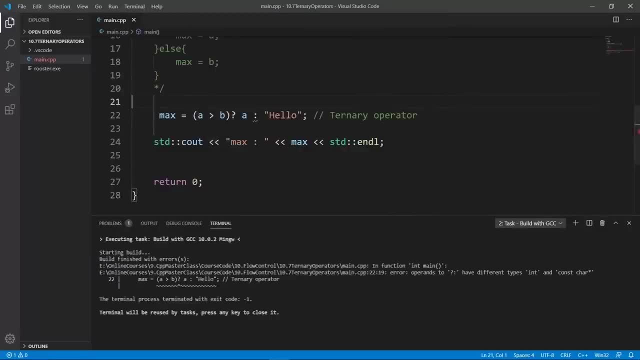 weld. we're going to also see an error from the compiler and it should be the same error. so operands to question mark and colon have different types and and cost car and they have to be stands. you can really compare. so, for example, we can take out this string here and put in a floating point. let's put in a 22.5 and say that this is a float. 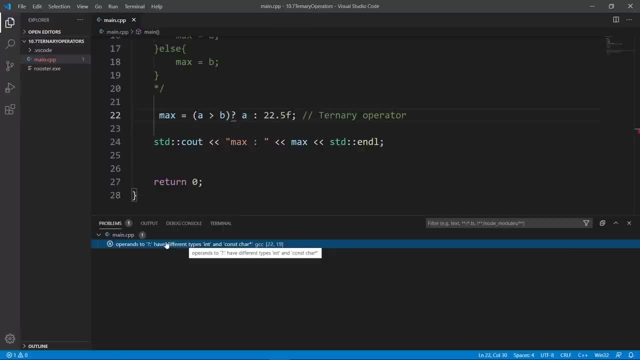 you're going to see that the problem is going to go away here. let's wait for a minute. it's not going away. we're going to build anyway. you see, the world is good, we're going to clear so that we don't have all this clutter. you see problems right away, and if we build again, let's. 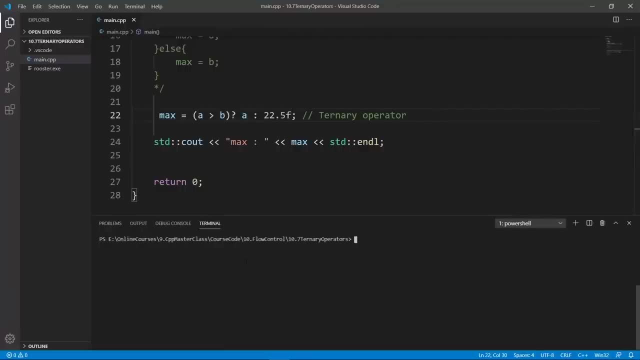 try to do that, the builder is going to go through and if we run this, we're going to get max is 22, because we are comparing a and 22 here and the compiler inserted an implicit conversion from this floating point to integer. that's why we are seeing this here. so what is the type that the 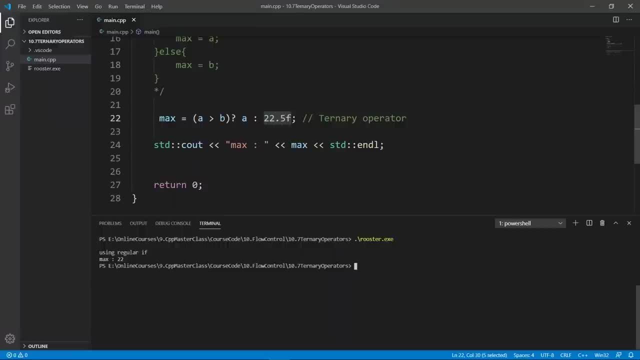 compiler really used here. okay, to make it really clear what is going on, we're not going to use max here. let's say auto max one and see what the compiler is really deducing to. so we're going to take this out and by this we're going to see what implicit conversion the compiler really did here. 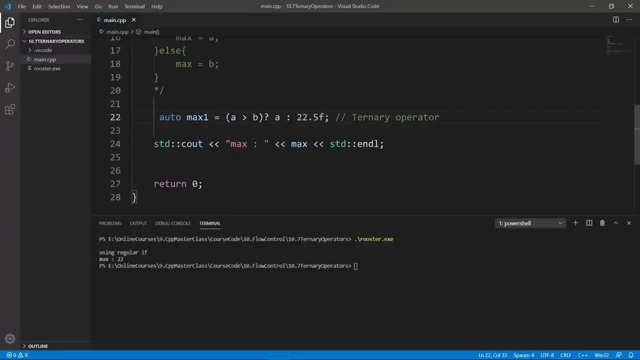 because what we had before we were doing an assignment- so whatever was on the left- was being turned into an integer. because we were doing an implicit conversion from an assignment. so whatever is on the left is turned into the type of whatever we have on the left of the assignment. i hope you know this already. 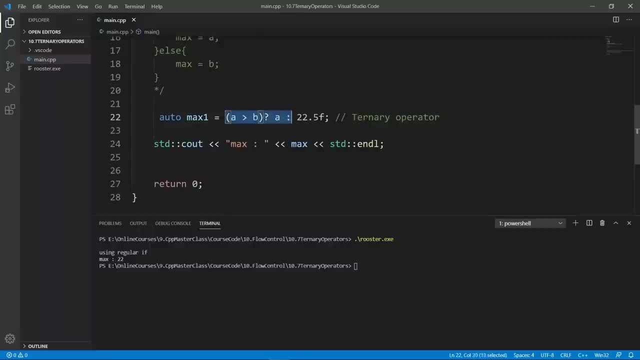 but if we do things like this, we're going to deduce whatever is on the left and assign that to max one. so we're going to do so. we're going to see the implicit conversion that the compiler did in here, and it is good to be able to see things like that. it is a curiosity thing. so 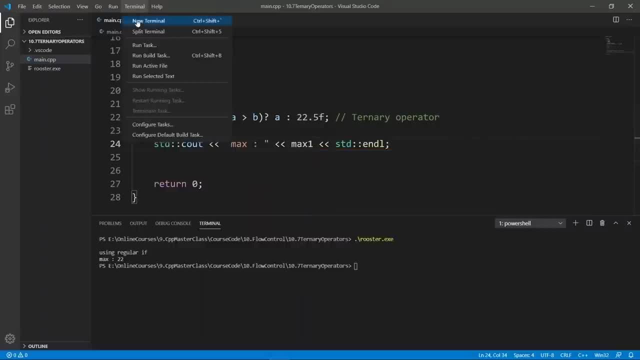 let's see what happens here. we're going to print max one and i'm going to world with gcc. this is going to go through and i'm going to see what is printed. so let's run rooster and you're going to see that the implicit conversion happened from end to float and we deduced the float here in max1. 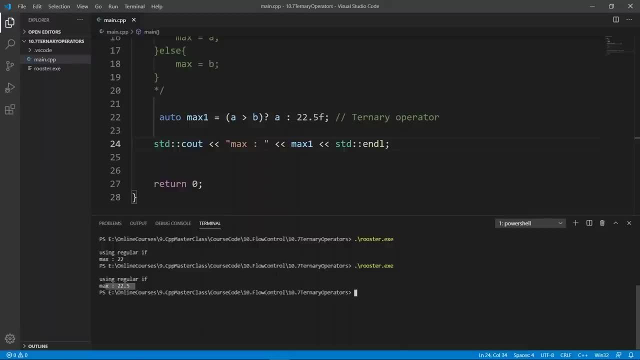 this is really interesting. one might have thought that we had a conversion from float to end, but it was actually the reverse, and this is quite interesting. this is really all we set out to do in this lecture. i hope you found it interesting. again, make sure you have this syntax here drilled. 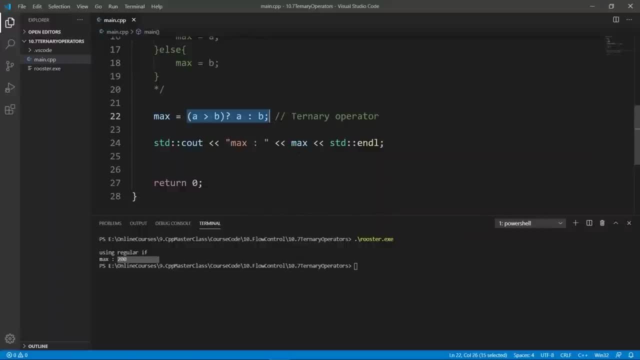 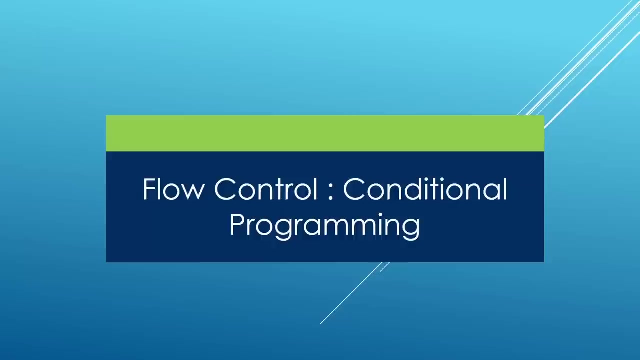 in your brain because you're going to be seeing this a lot in your career as a software developer- not only a c plus plus developer, actually- and it is going to be helpful for you to know this- the change in your rapidly classifying you will see more signage in your cloud strings. 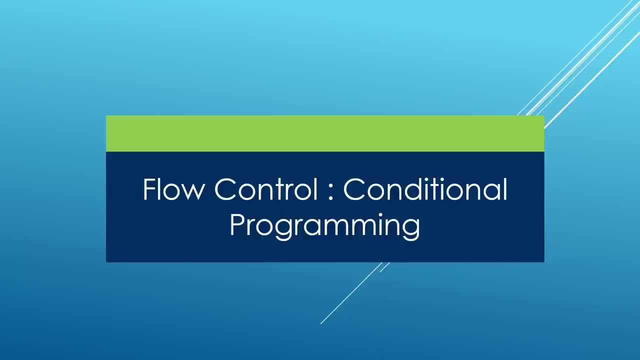 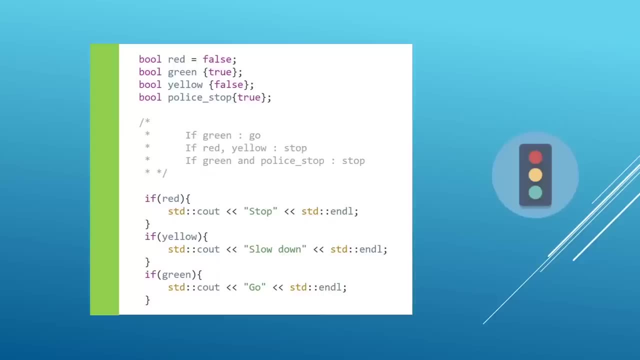 more stark messages and so on. we had an opportunity to talk with these 5 different software developers and we were able to see all kinds of three-post software development features. one was around the learning seconds after the first, after you started learning ele chunks of, yeah, the execution. 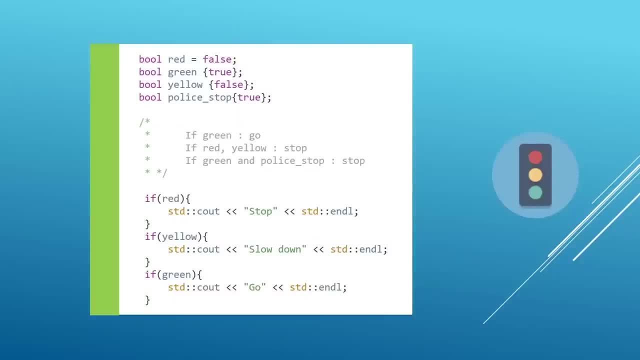 data kind mineral old data was really part of this click through which you will see that's basically supplementary learning Zach — 🎶, that goes 포 was my success rate on this chapter. this chapter was all about flow control and we had the chance to learn about many of the tools that C++ provides to deal conditional programming, and we were about to see. 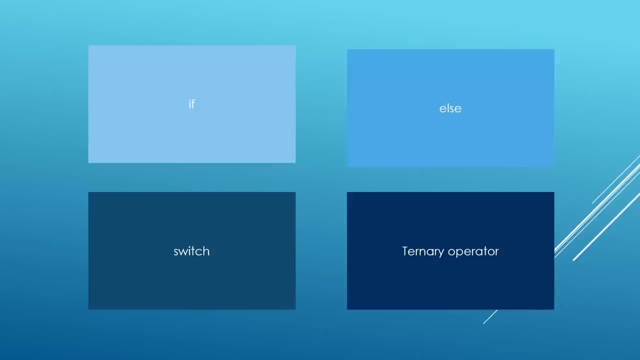 plus, plus provides really revolve around these four things. here we have if statements we can do else, closes on these if statements we can do else, if to really do long chains of thanks where we do different decisions to do things in our applications, we also saw that switch is an. 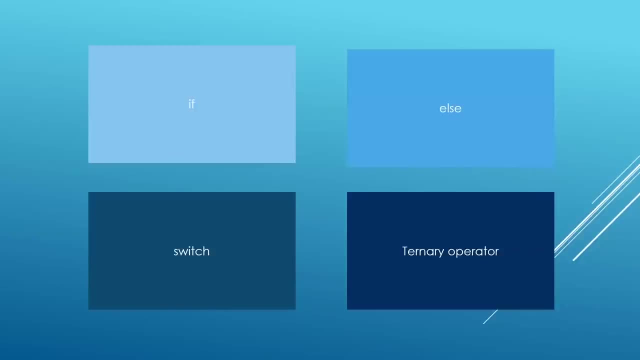 option if you have several decisions you can make in your application, and we saw that a ternary operator can really be used to do two decisions. if you have two decisions, you're going to be able to reduce the number of lines you use to do these decisions with to one line, and we had a chance to. 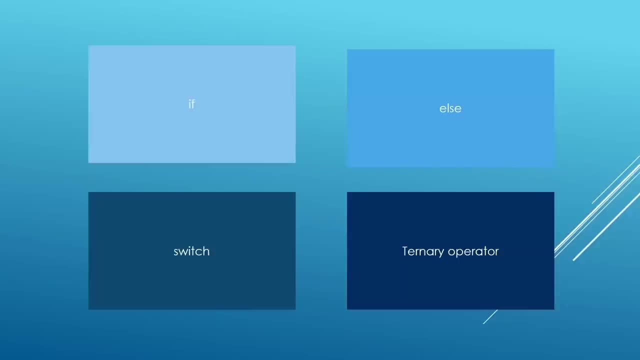 really look at that in detail in the lecture on ternary operators. this is really all i had to share in this chapter. i hope you found it interesting. we are going to stop here in this lecture. in the next chapter we're going to start and learn about loops. go ahead and finish up. 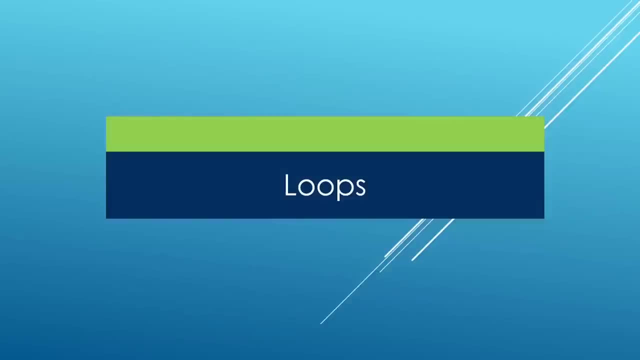 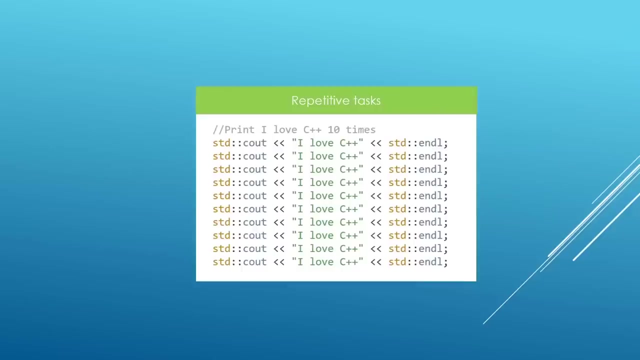 here and meet me there. in this chapter we're going to be learning about loops, and this is a construct that is provided by the c plus plus programming language to allow you to do repetitive tasks relatively easily. suppose we have a task to print a message 10 times. we can go down and 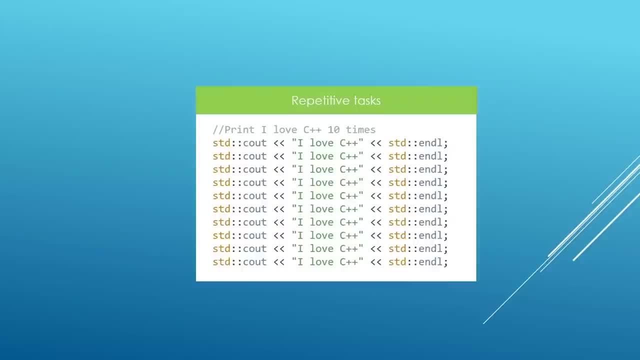 do it like this and it is going to work. but what if they try and tell you: do this a hundred times? then you're going to start scratching your head, you're going to type this a hundred times and you're going to run your program and it is going to work. then your manager comes up and they say: 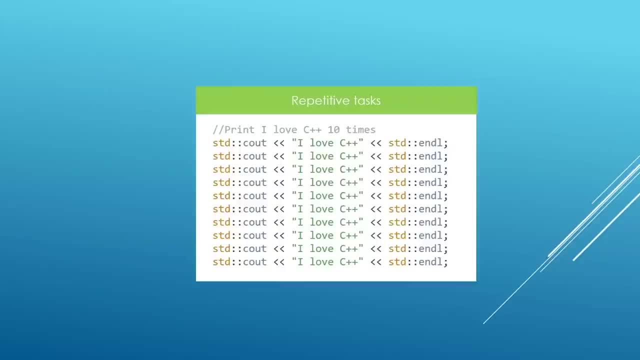 i want you to do this 10 000 times, or even 100 000 times. so then you're going to start pulling your hair or running around breaking things, because that's impossible to do. not to worry here. c plus plus provides a way to do this relatively easily, and we're going to be learning about ways. 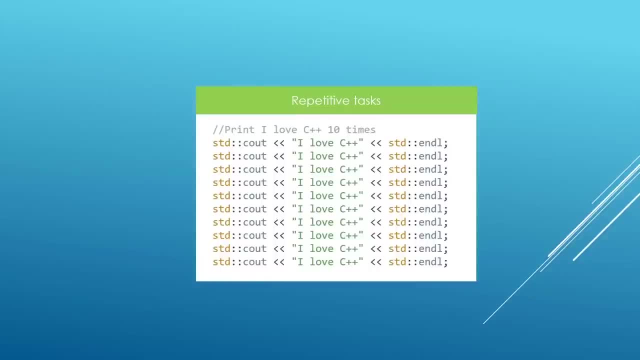 we can do this in our program in this chapter, the constructs we're going to learn about ways we can do this in our program, in this chapter, the constructs we're going to be using are these: you see, here there is a for loop, a range based for loop, a while. 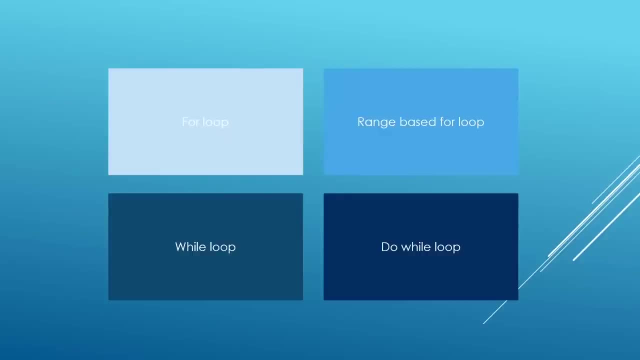 loop and do a while loop, and we can make use of these tools to not go crazy printing a message one million times, because that's really bad, okay, so that's what we are up against in this chapter. we're going to be learning about these loop constructs and you're going to find that they 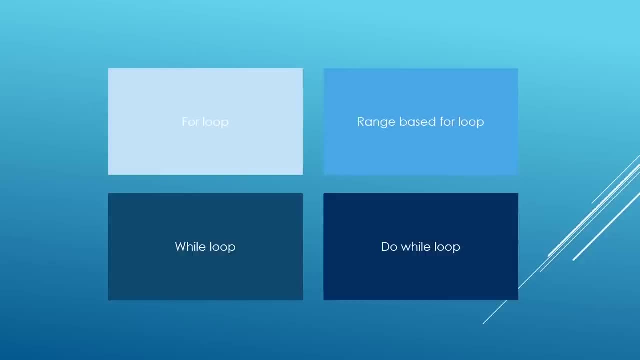 are really cool for your application. i am excited to be teaching you this, so let's get started in the next lecture, and we're going to be learning about how to do this in this chapter. so let's learn about the for loop. go ahead and finish up here and meet me there. in this lecture, we're going 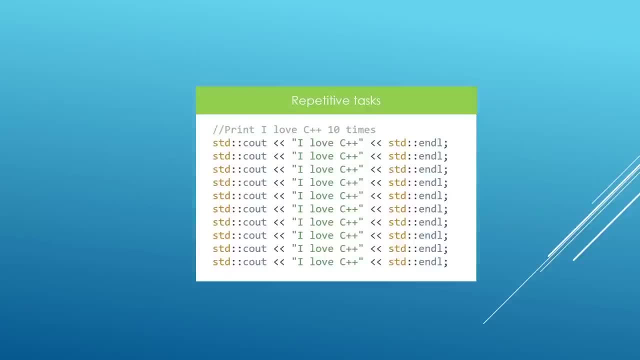 to learn about four loops. four loops are one of the constructs we have in c plus plus to do repetitive tasks. they allow us to do something like this much more easily. for example, we don't have to type stdc out. i love c plus plus. 10 times or 100 times, we can do this in less. 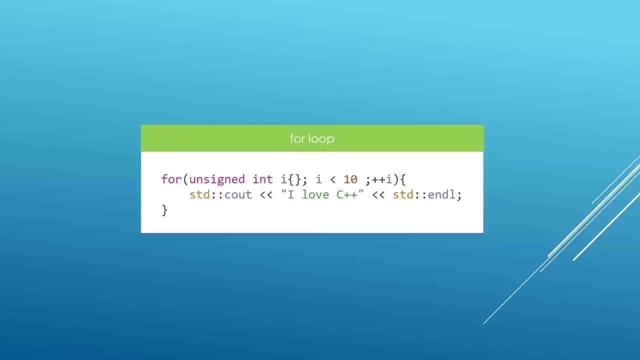 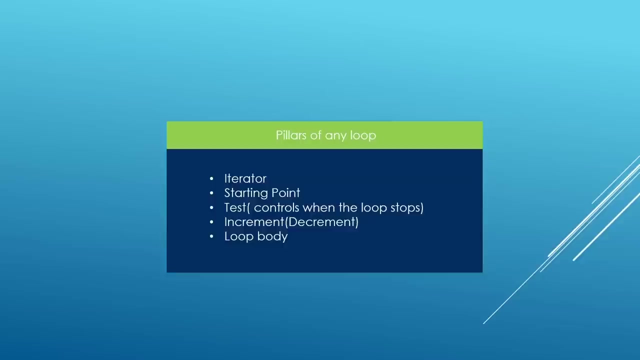 than five lines, and you're going to see how cool this is. the syntax for four loops is going to be very simple. it's going to look like this and, uh, it may look intimidating for first users, but we're going to break this down. we have a few parts in here. the first part is the iterator, which is a 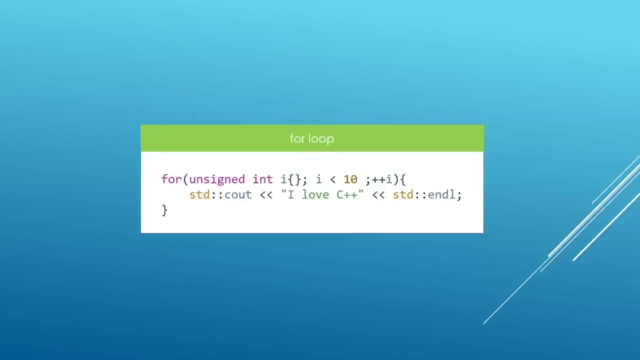 variable that we're going to be using to navigate through the loop, and that variable is this unsigned int i. here we are going to initialize this to 0, and the value we initialize this with is going to be our starting value, and that's another key point of this tutorial. 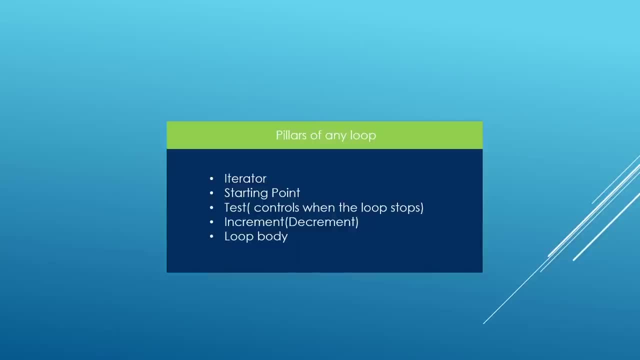 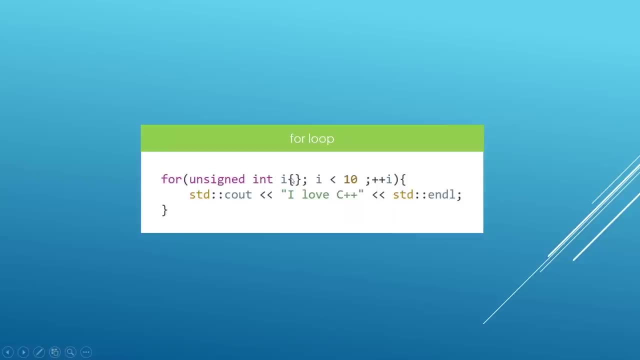 we are going to have a test which is going to control when our loop ends. for example, this loop is going to start with i, equal to 0. it is going to keep doing stuff until i is no longer less than 10. as long as i is less than 10, it's going to keep doing whatever it is we want to do, and the first 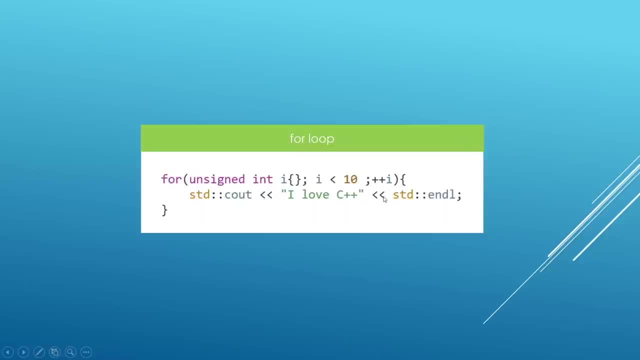 part of the loop is this: plus plus. i thing here, and this is an incrementation part, that's going to be the first part of the loop, and then the second part is going to be the last part of the loop, and that's how i'm going to call it for simplicity, but it leaves a part that keeps. 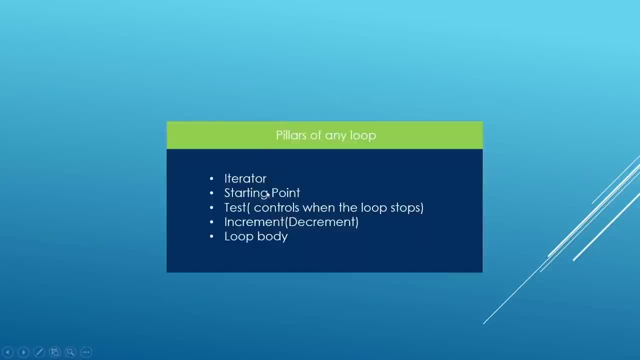 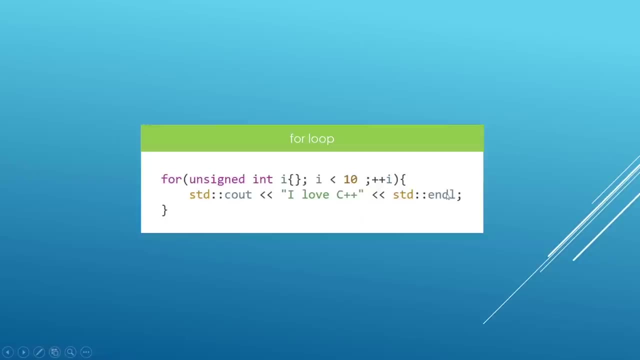 changing our iterator to make our loop move forward. after these four points, we are going to have a pair of curly braces and inside these curly braces we're going to have the body of our loop and this is the code we want to execute multiple times. and inside this loop body we can really do. 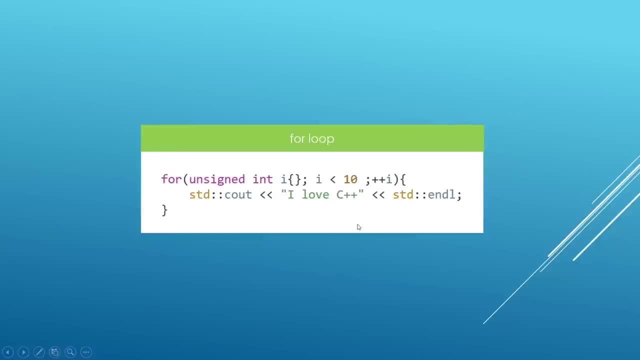 all kinds of crazy things. you're going to see how cool this is. again, we have a few parts with our iterator, which is this variable i. here we're going to be initializing this with a value that denotes where we want our loop to start. we then have a test which is going to control when the 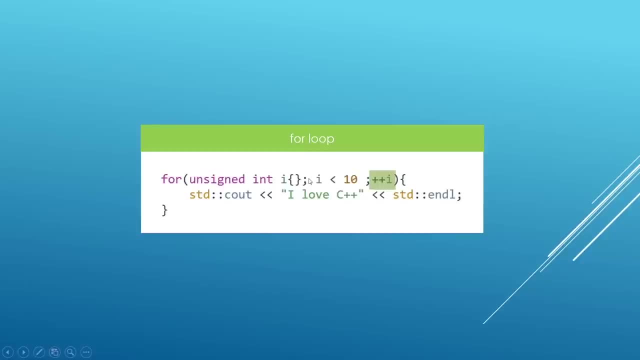 loop is going to end. we're going to have our incrementation part, which is going to allow our loop to move forward, and it's going to be doing that through incrementation or decrementation. but to make explanation easier here, we're going to call this part the incrementation part of the loop. 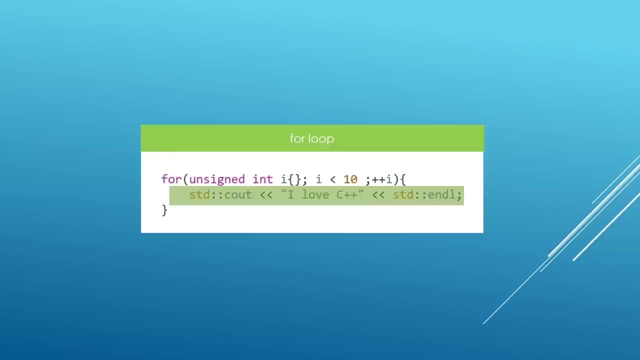 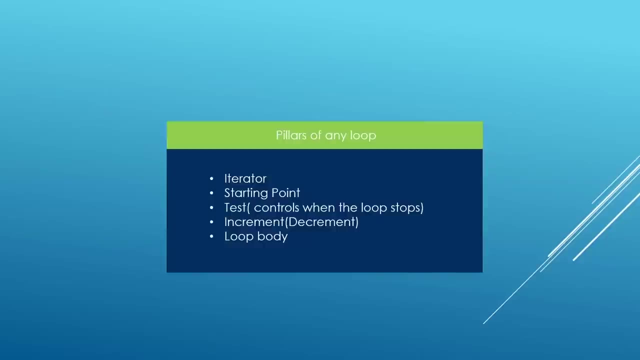 so we're going to have the body of the loop and it's going to be within these curly braces and it's going to be whatever it is we want to execute inside this loop. okay, these are the parts of a loop and you need to keep this in mind. okay, now that you know the main parts of a loop. 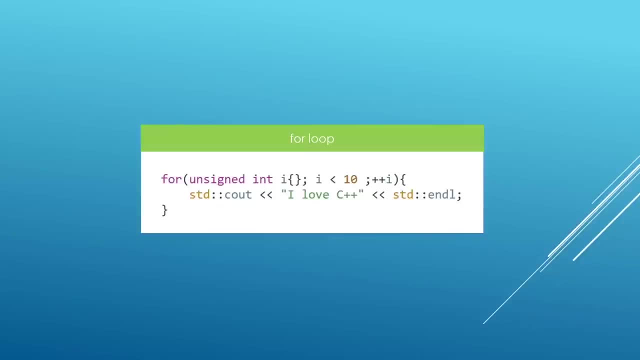 how does it really work? let's go through this and see how it's going to print. i love c plus plus 10 times. so when this code gets executed, we're going to start with i equal to zero, because that's what we are initializing this value with. 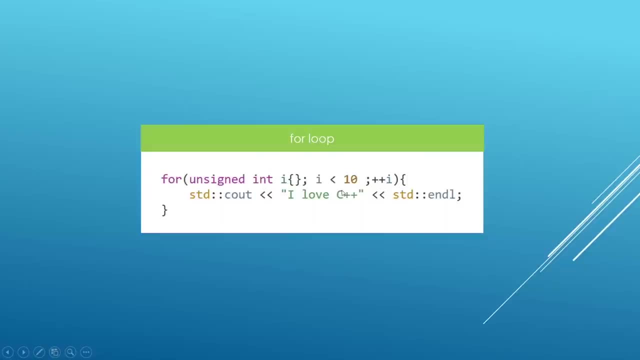 after the incrementation part, we're going to run the tests and the test is going to say: is i is zero less than 10? and that's going to be true. so if the test turns out to be true, we're going to jump into the loop body and if it's false, we're going to jump to the end of the loop and execute. 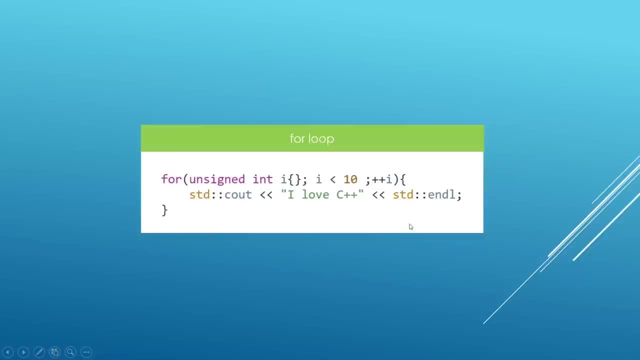 whatever is after our loop. this is how it works. so if we jump in for the first time when i is zero, we're going to print i love c plus plus for the first time. then, after the body is executed, we're going to execute the incrementation part. 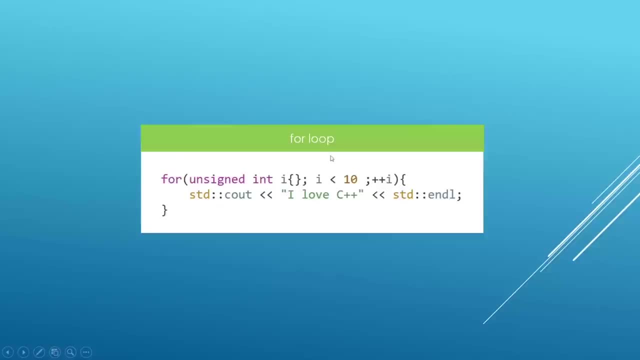 this is going to make i equal to 1. then we're going to come back to the test. we're going to say: is one less than 10? that's going to be true. we're going to come in the body and print: i love c plus plus for the second time. after that, the incrementation part. 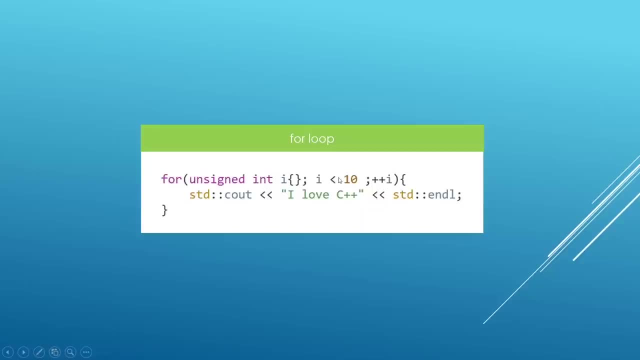 is going to run. we're going to have a two inside i here. two is less than 10.. this is going to be true. so we're going to fall in the body again and print: i love c plus plus for time. we're going to keep doing this until we hit 9, for example, if we increment and get a 9. 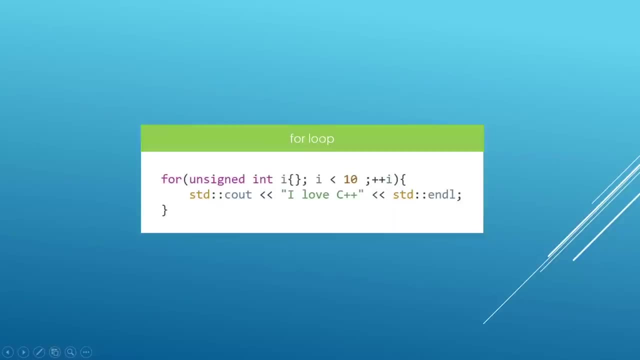 we're going to fall in the test and say: is 9 less than 10? that's going to be true. so we're going to fall in here and print i love c++ again, and after that we're going to run the incrementation part again. this time i is going to become 10. we're going to do the test: 10 is not less than 10. so 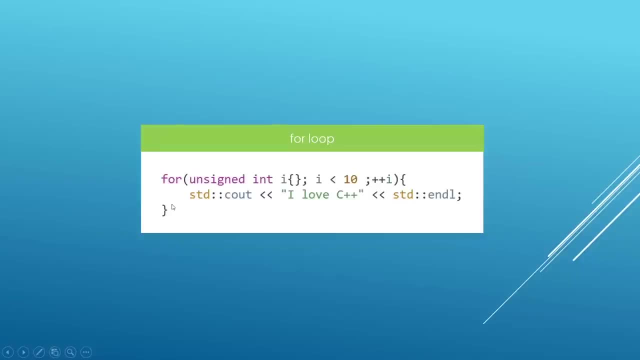 the test is going to fail and we're going to fall on the outside of the loop here and by that time we will have printed i love c++ 10 times, and this is really how a loop works. for the first time, we're going to run this initializer part here to initialize our iterator, which is this value: i. 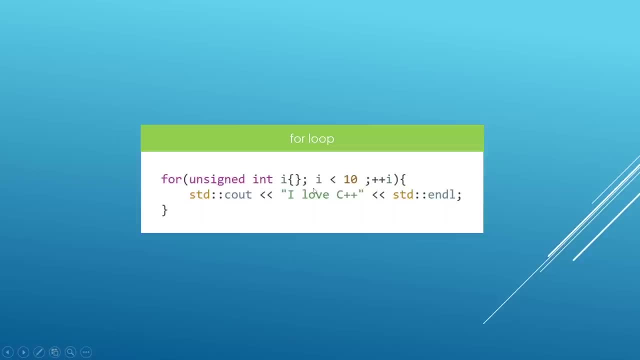 and then after that we're going to run the test. if the test is good, if it's successful, we're going to fall in the body, we're going to execute whatever code is in the body and after that we're going to keep doing the cycle- increment test body, increment test body, increment test body- until we hit a point where 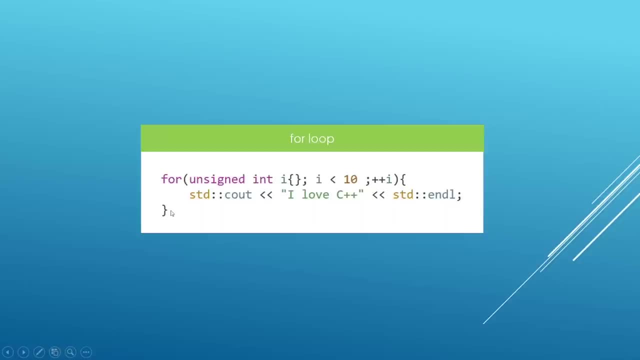 the test fails. and if the test fails, we're going to fall outside this for loop. here. we're going to execute whatever is after this close-in curly brace, and this is how a loop works. i want you to go through this one more time by printing: i love c plus plus and making sure that this is. 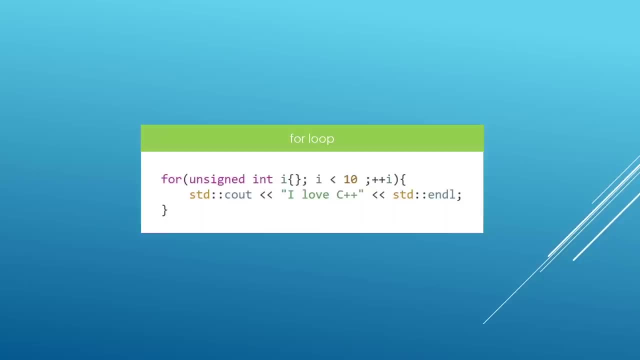 printed ten times, and one thing you should have noticed now is that we use this test to control how many times the loop is going to start, for example, if we wanted it to run an example thing. the main important thing is to understand how loop works. one thing i want you to notice: 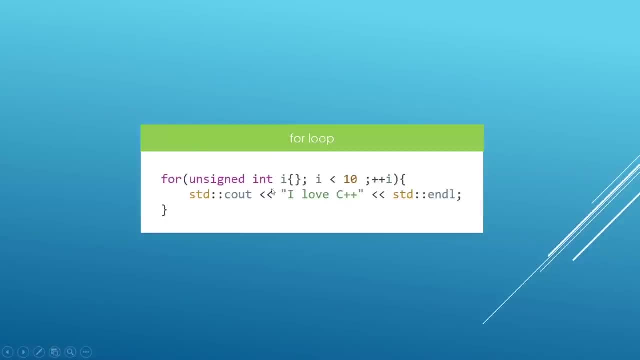 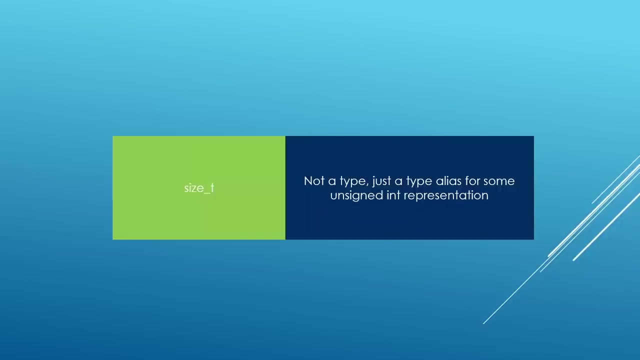 is that we are saying unsigned int here to declare our iterator. iterators are a common thing in c++ code and they're not just used for loops like we are doing it here. there is a type we use to do iterators and it makes our code much more readable, and that's called size t, this thing. 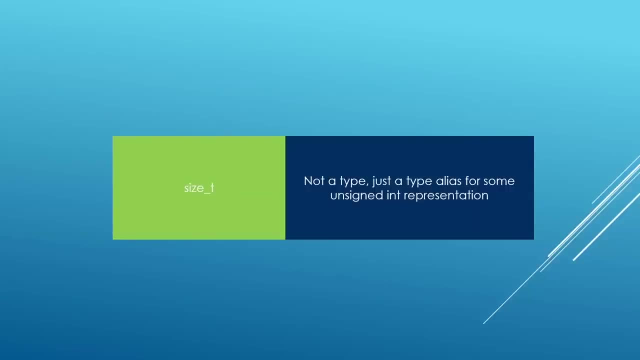 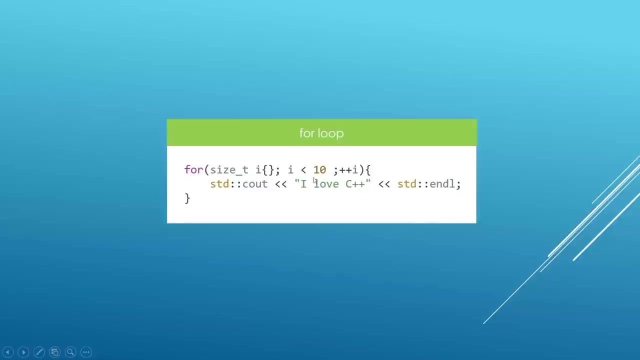 is a representation of some unsigned int type in your c++ compiler. this is going to be different from compiler to compiler, but for example, on my system this is eight bytes, so it has quite a good range of values you can put in there. if we use size t type to declare our i iterator, here we're. 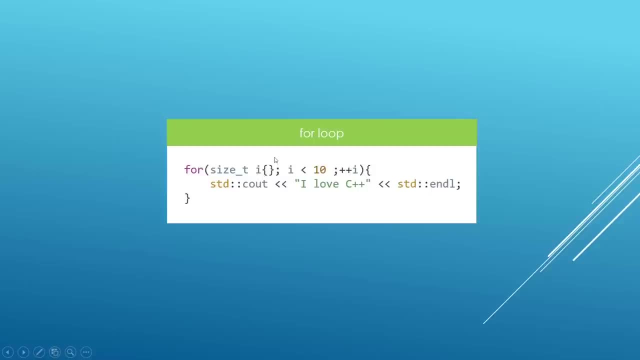 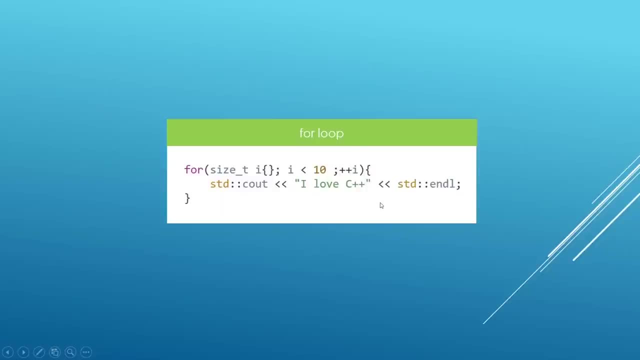 going to put our incrementation part and i think i really emphasize this. but the parts of our loop inside this parenthesis are separated by semicolons like this: so we have the iterator declaration, we have a semicolon, we have the test, we have a semicolon and we put our incrementation part. 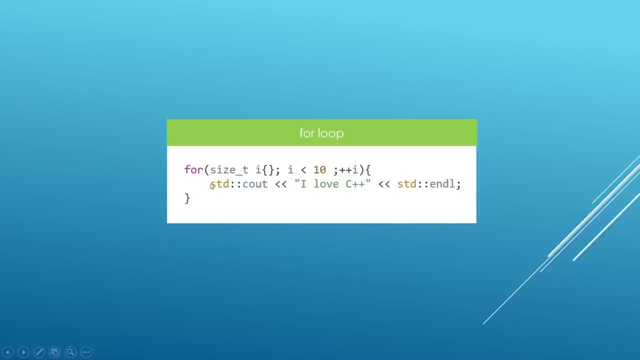 and then we go on and put our curlies and inside we can do whatever it is we want to do inside the loop. so size t is something you're going to see a lot. make sure you know what it means. remember that it is a representation of an unsigned and type, so it can only represent positive numbers. 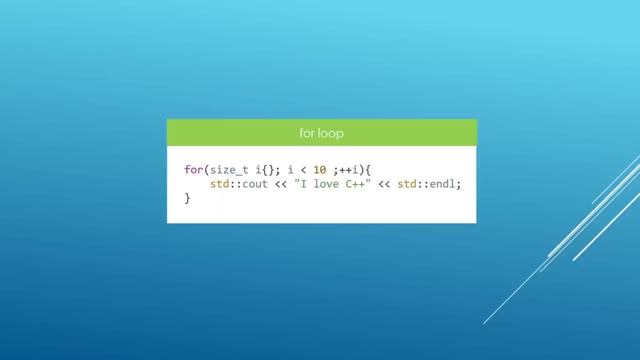 and it is used to represent things like sizes in c plus plus thank, the number of students in a classroom, for example. that can never be negative. think about the number of seats in a car. that's something that is always going to be positive and it won't make sense for that. 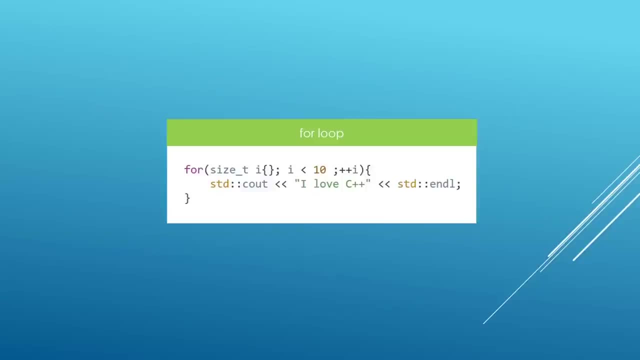 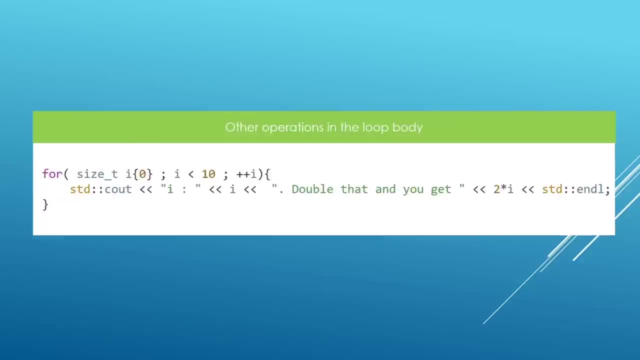 too, be negative. so for those kinds of things, we can use size t to represent the size of those things, and you're going to see how this works in a minute. okay, now that you have a pretty good idea about how a loop works and the main parts that make it up, i want you to know that you can also do. 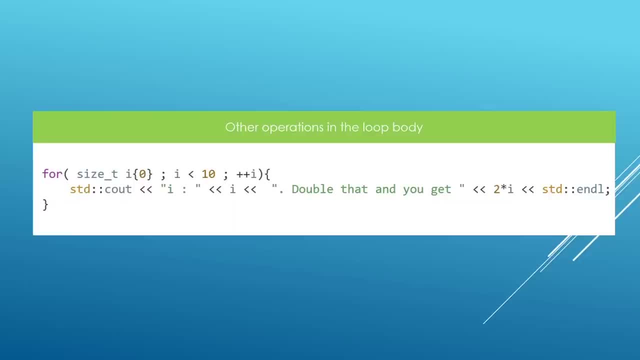 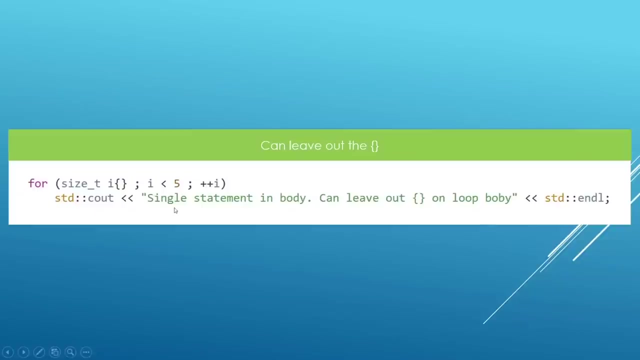 all kinds of crazy operations inside the body of your loop. for example, here we are printing out the current value of our iterator and we're going to print the double of that. we can do this. we can also leave out the curly braces, and this is only valid if we have one statement we want to run in. 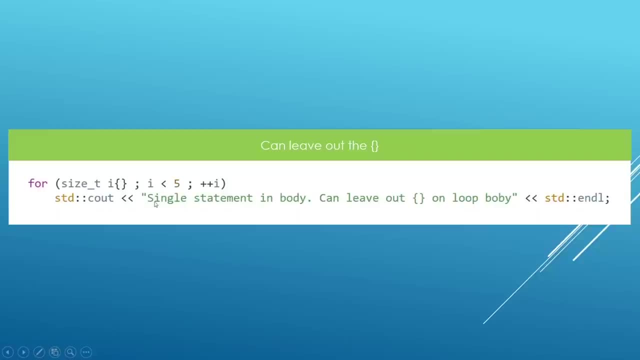 the loop. so this is going to print this message here five times, because this loop is going from zero all the way to four. it is going to stop when i stops being less than five and this is going to be five times. if you go through this, you're going to see that this is going to print five times. 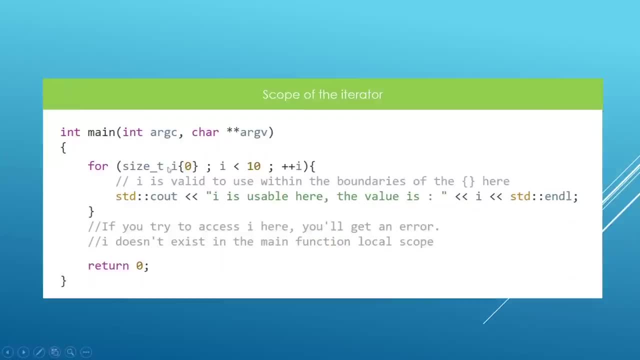 you should also know that this iterator that we are declaring like this is going to be scoped in the body of the loop, so you can only use it inside these curly braces. and if you try to use it outside, for example here, after the closing curly braces of the body of the loop, you're going to get. 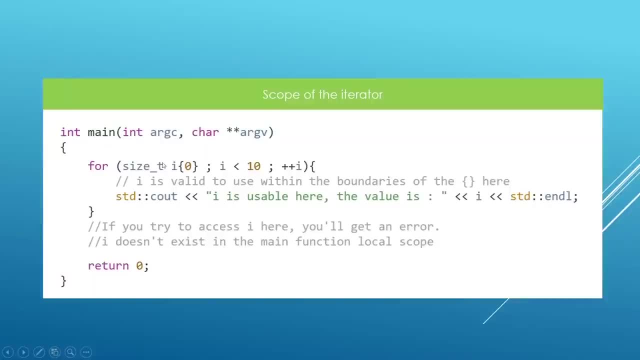 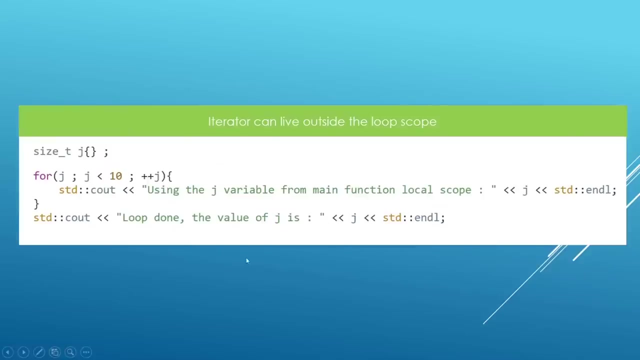 a compiler error. again, you can only use this variable i, which is our iterator, inside the curlies that mark the start and the end of our loop body. if you want the iterator to be usable outside the scope of the for loop, you can do something like this: you can declare your iterator outside the loop and you can. 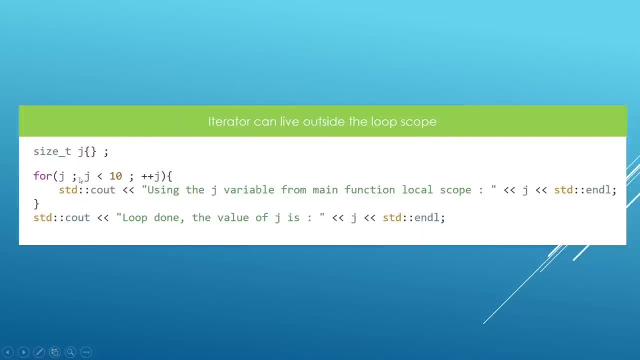 initialize that with whatever you want and then you can set up your loop like this: you can say for j and put in your test and your incrementation part and inside do whatever it is you want to do in the body of the loop. if we do it like this, then j is going to be usable outside of the loop and 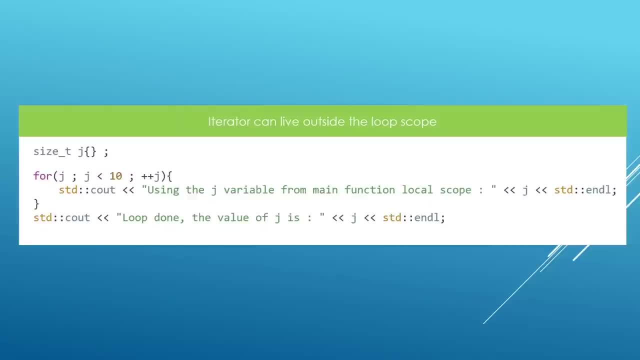 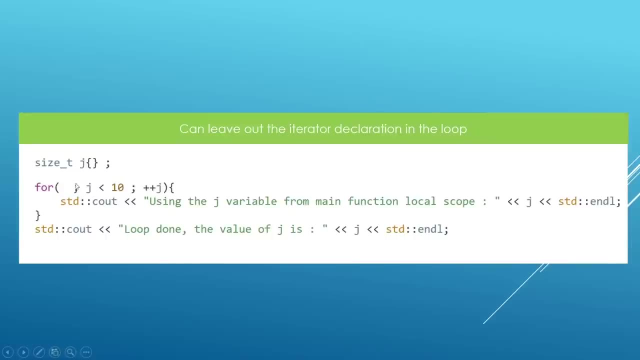 we're going to see its value if we print it out like this. so this is also something you can do. you can even go all crazy and leave out the declaration part if you happen to have the iterator declared outside. so if you do something like this, it is also going to work, okay. the last thing i want you to see: 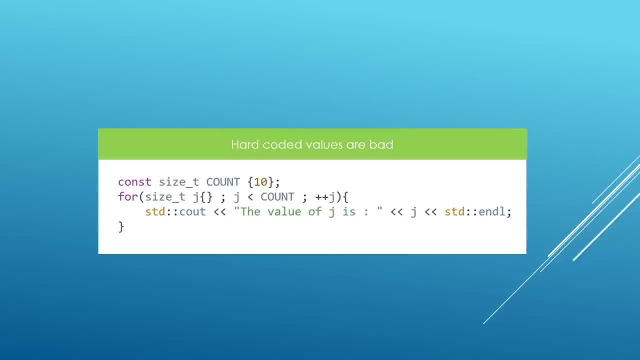 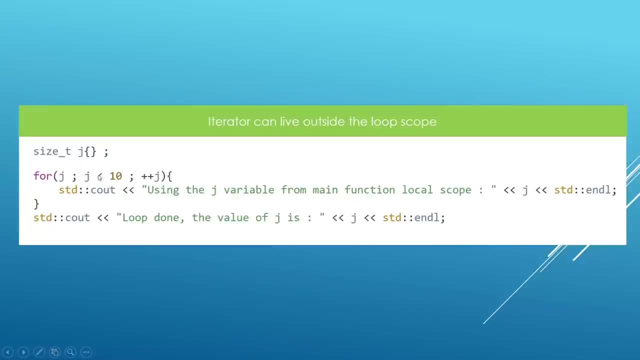 before we head over to visual studio code and actually try this out, is that it is a bad thing to hard code your values in, for example. you see here we are saying j less than 10. this is really bad design because every time you need to change the number of times that your loop is going to run. 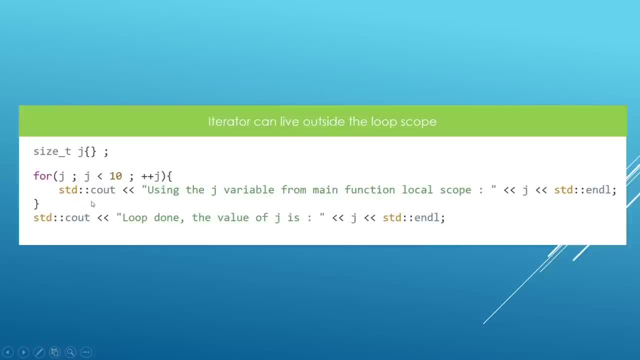 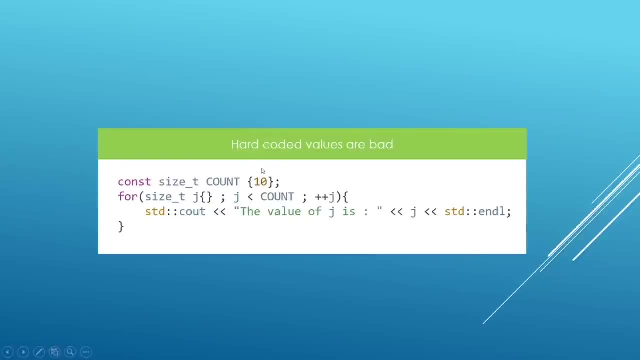 you're going to have to hunt for these loops and change these values, and this may be in a lot of places in your code, so a good thing to do is to put the value that controls how many times your loop is going to run in a variable like this. we're going to store that value in. 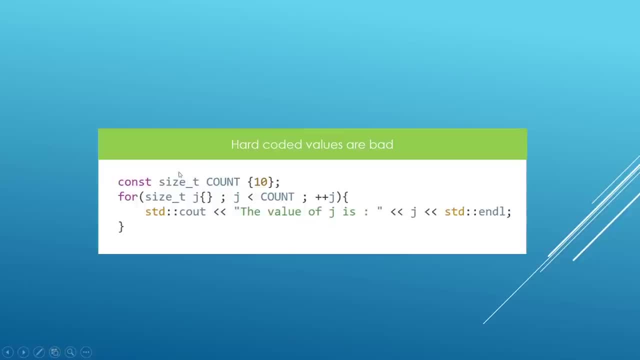 this count variable. notice that it is of size t because it is a representation of the size of things, something we don't really want to be negative, and we're going to use the in our test part of our for loop here. instead of saying j less than 10, we're going to say j. 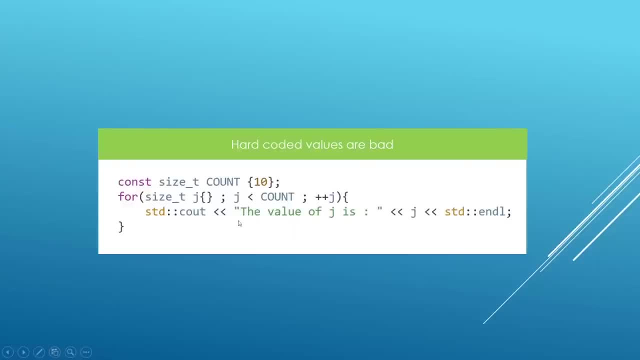 less than count, and if we want to change this, we have one point of control to go and change this value here, and this is really good design. you should do this, okay? we have talked a lot about loops. it is time we headed over to visual studio code and actually tried these things out. here we 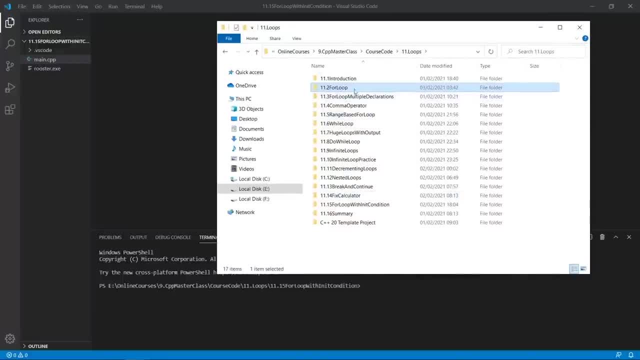 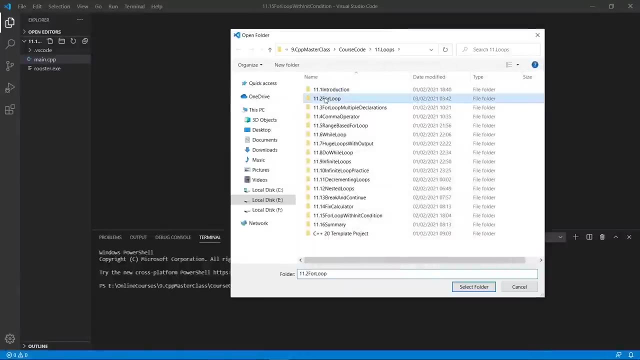 are in visual studio code. the current project is for loop here. we're going to grab the code from our template project and we're going to put that in place here and we're going to open this in visual studio code. so let's do that pretty fast for loops. that's the current project we. 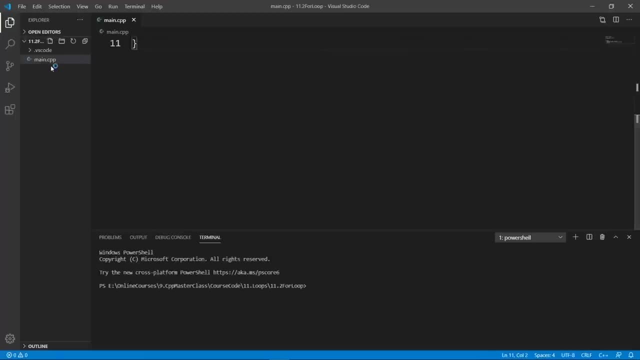 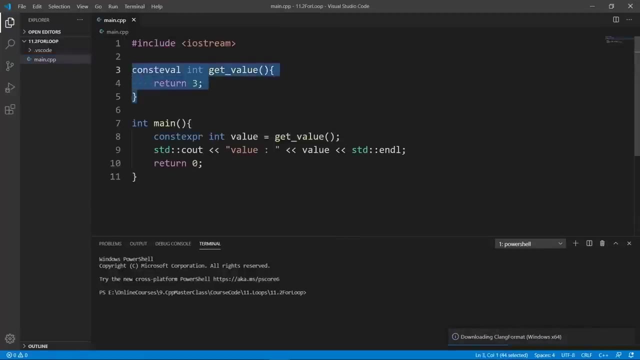 select it and we open this in visual studio code. we're going to open up our main cpp file, which is going to show up here, and we're going to remove things we don't need here. so let's remove that, okay. the first thing i want you to do is the bad way to do things. 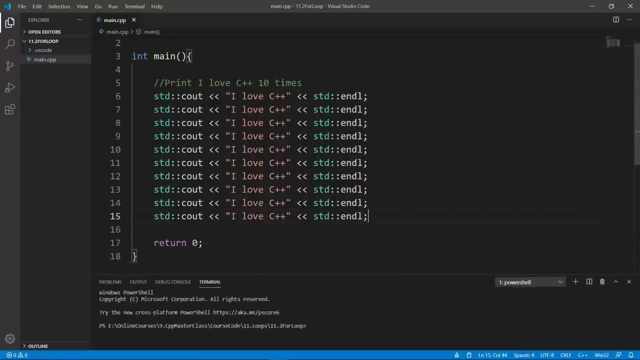 again, if we want to print- i love c++ 10 times- we can do it like this and if we run the program it's going to work. but this is really bad design because you would have to copy and paste this, for example, a thousand times or even a hundred thousand of times, and that's really bad. so if 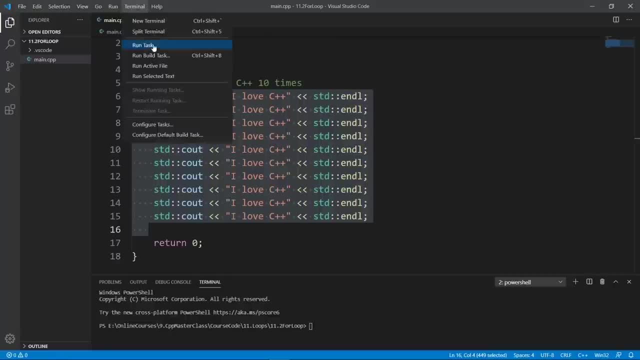 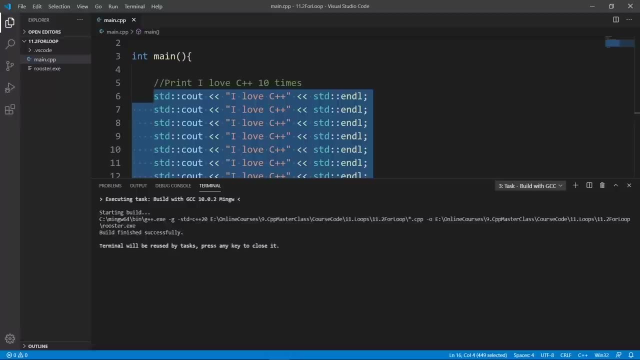 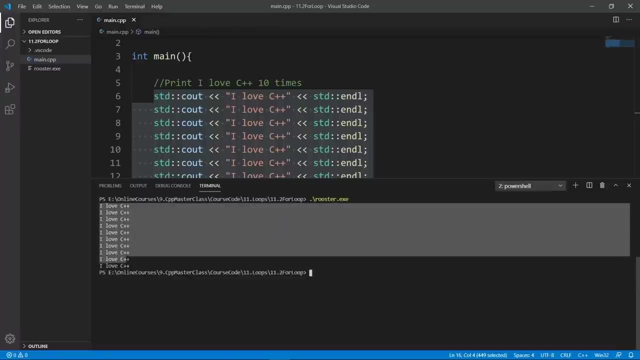 we bring up our terminal and build with gcc, like we always do. you, the build is going to go through. you see, it's successful. we're going to clear and we're going to run rooster and it's going to say: i love c++ 10 times. if you count this, it's going to be 10. 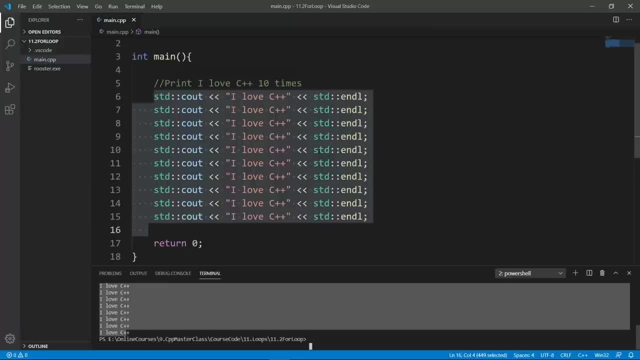 times because that's what we're doing here, but this is really bad design. you don't want to do something like this, so we're going to comment this out and do this better using a for loop. let's say that this is the bad way and we're going to use for loop, which is the good way. sorry, 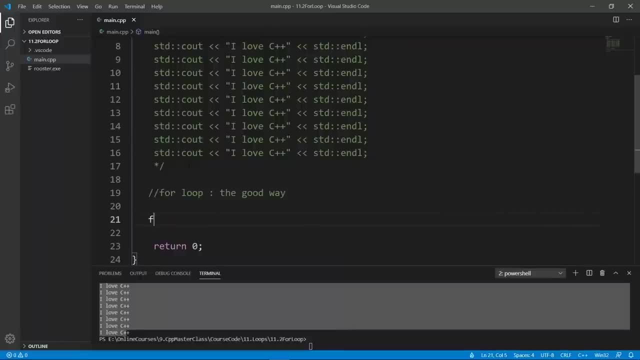 so we're going to start by declaring our iterator. so we're going to say for. we're going to say size t, let's use unsigned, and to show you that you can use that. and we're going to say i, and we're going to initialize this. 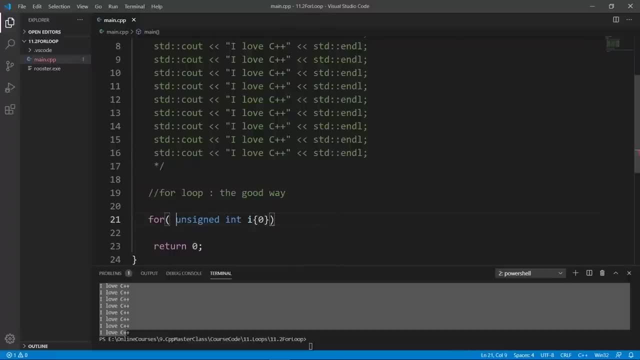 with a zero, and this is going to be the declaration of our iterator. this is the first part we have in this parenthesis. here we're going to put in a semicolon and put in the test. we want the loop to run 10 times, so it's going to run from zero to nine. we're going to stop. 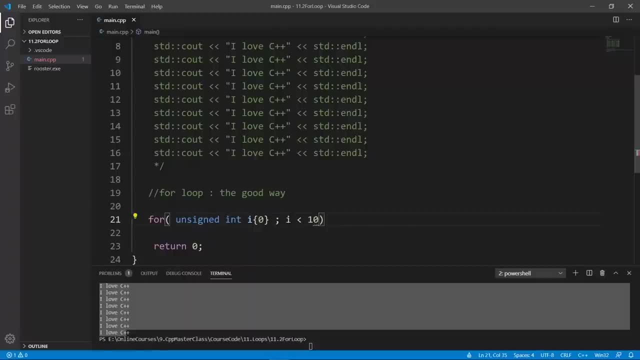 when i stops being less than 10.. this is one way you can understand this. after we have our testing, we're going to put the incrementation part, which is going to change the iterator to make the loop move forward, and we're going to do that by incrementing our iterator. after that, we're 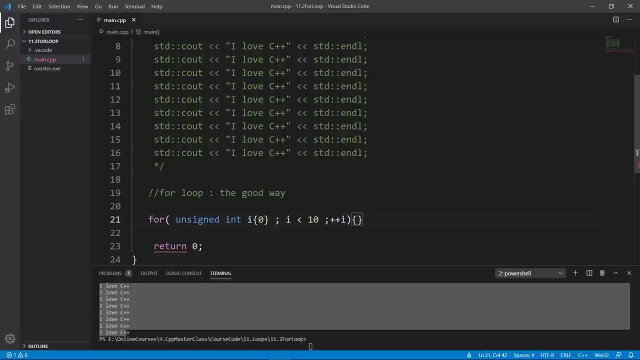 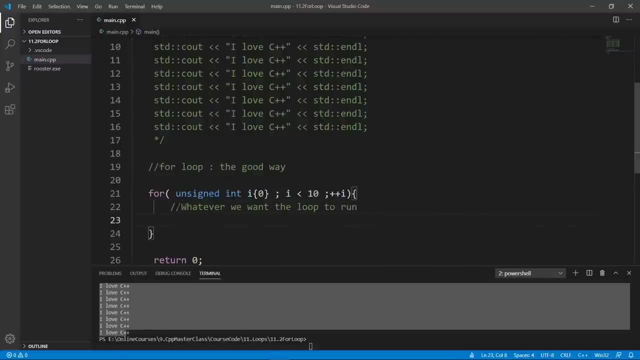 going to put a pair of curly braces- not angle brackets- and we're going to fall inside the body of the loop. this block here, delimited by the curly braces, is the body of the loop and we're going to put whatever we want the loop to run, so we can go down here and say i love c plus plus 10 times. 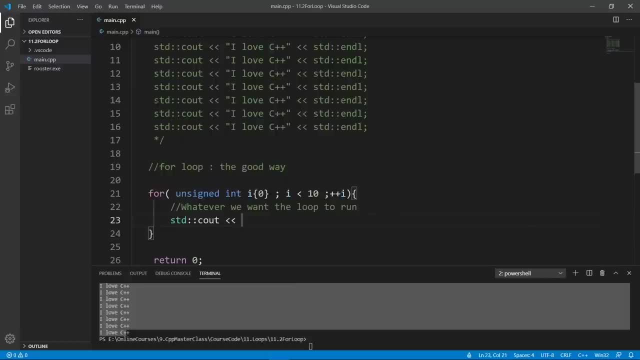 let's say that. but before we do that, let's say i, so that we know the current iteration, where we are at, and we're going to put a column and say i love c plus plus. this is going to be better to follow in the terminal, i guess, and we're going to put in our new line character. move to the new line. 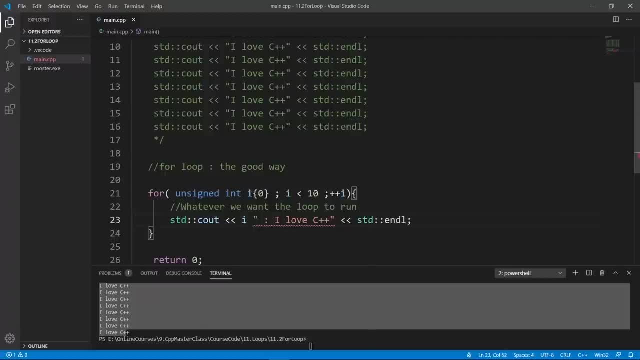 and we're going to put in our new line character and we need to put our stream output operator here for this to make sense to the compiler. and this is our loop now, if we run it, we're going to see exactly the same thing like this, but we're 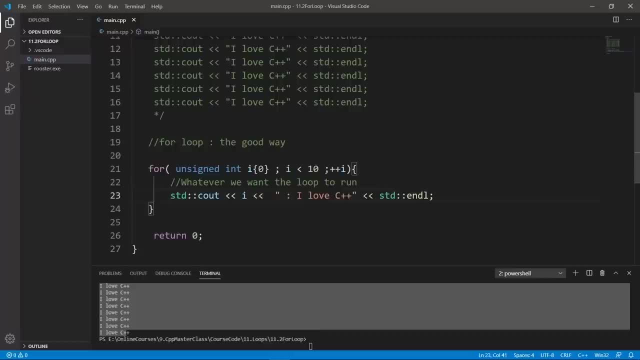 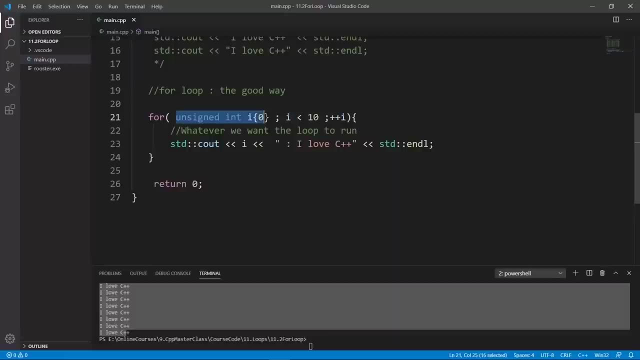 going to have these iterators prepended to the message so that it becomes easy to follow this and again how this is going to work. we are going to run our code to declare and initialize the iterator. after that we're going to do the test. we are going to start. 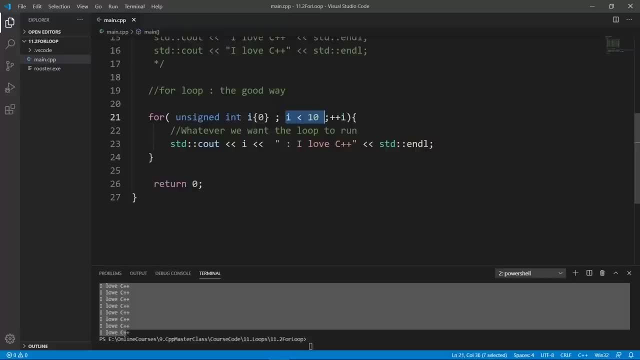 with i: 0, so 0 is less than 10.. this is going to succeed. we are going to fall in the body here and after that we're going to print stdc out. i love c plus, plus, and this is going to be 0. 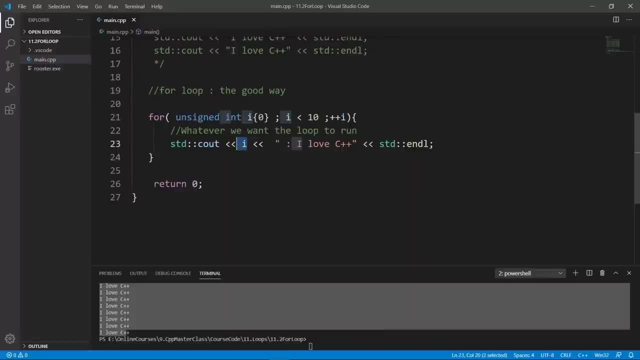 we're going to increment i and we're going to do the test again. we're going to have to do is one less than 10.. the test is going to be successful, so we're going to fall in here and we're going to print a one and we're going to run the incrementation part again. we're going to 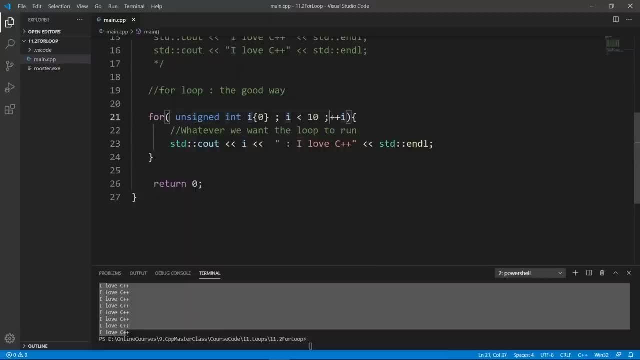 test, and we're going to keep doing this until we hit a point, for example, when we increment this to be a 9.. and after that we're going to run the test we're going to say is 9 less than 10.. the test is: 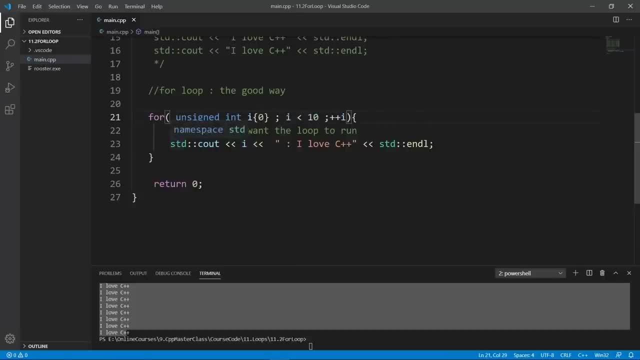 going to be successful. so we're going to fall in here and we're going to print 9.. and after that we're going to increment again, we're going to run the incrementation part and we're going to make i a 10.. if we run the test we're going to say is 10, less than 10.. the test here is going to fail. 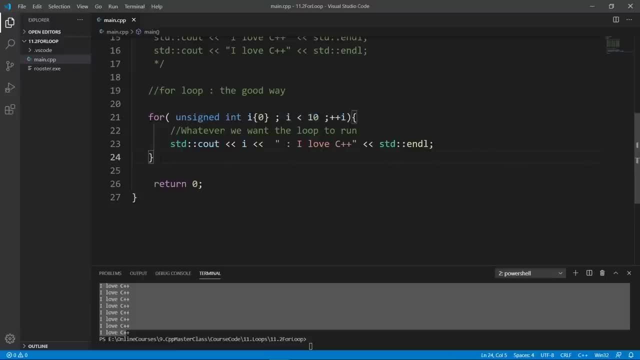 altogether and we're going to fall on the outside of the loop and say: loop done. let's say that so that we can see this on the terminal and this is going to run and print: i love c plus plus 10 times and we expect i to go from 0 all the way to 9.. try to run this in your mind. take a piece of paper, try. 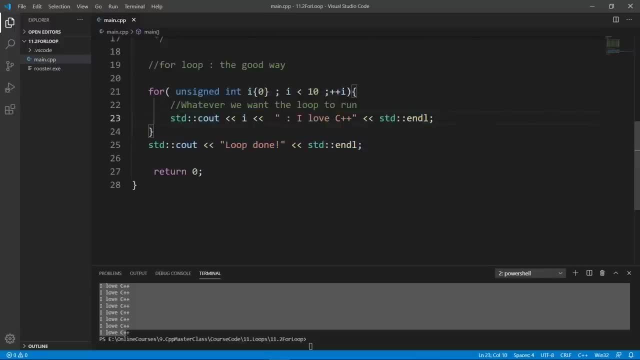 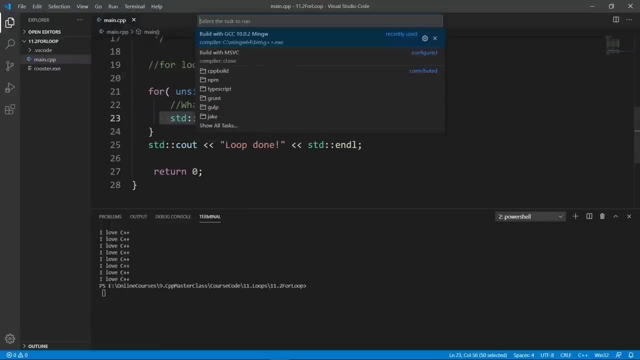 to print this as you fall into the body of the loop. you're going to see that's exactly what is happening here. so what we're going to do, we're going to weld this again. so we're going to run the task to build with the gcc. the world is good. we're going to go down and 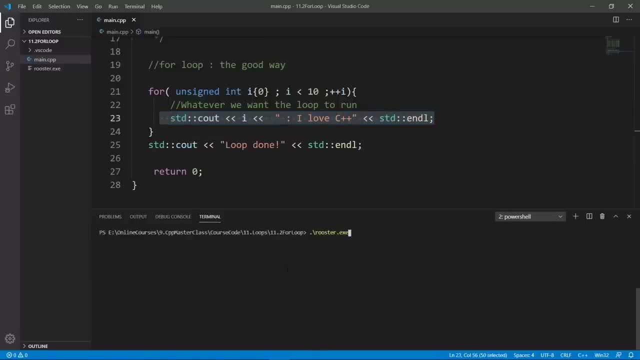 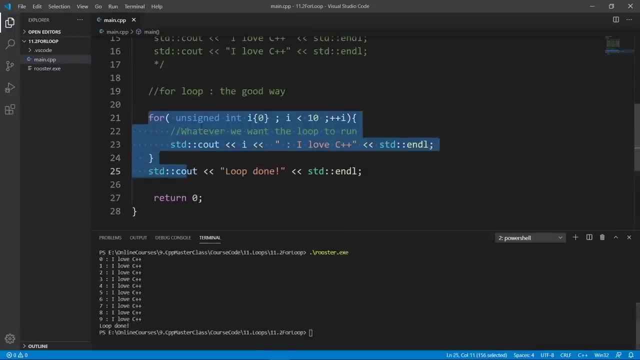 run this. we're going to clear and run rooster and you're going to see that we have a zero. i love c plus plus all the way to nine. i love c plus plus. our loop is working exactly the way we want. okay, so this is the first step. we are able to run our code a lot of times without really having to. 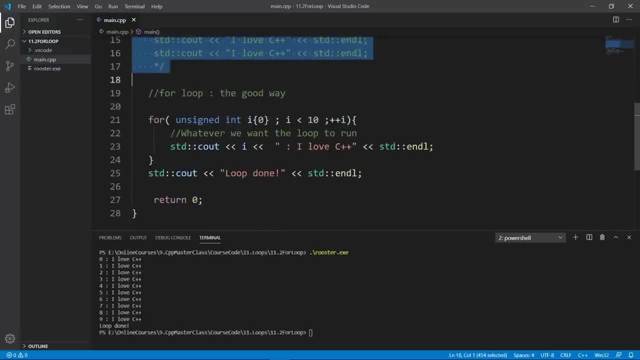 manually do things like this, and the benefit of this is that if we want this to run, for example, 100 times, all we have to do is change our test to go until i is equal to 100, and we're going to stop when i stops being less than 100. and if we 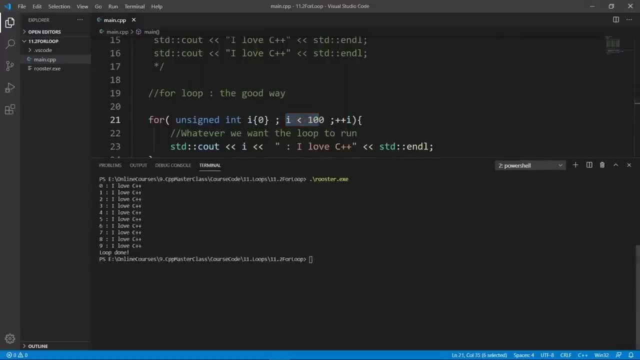 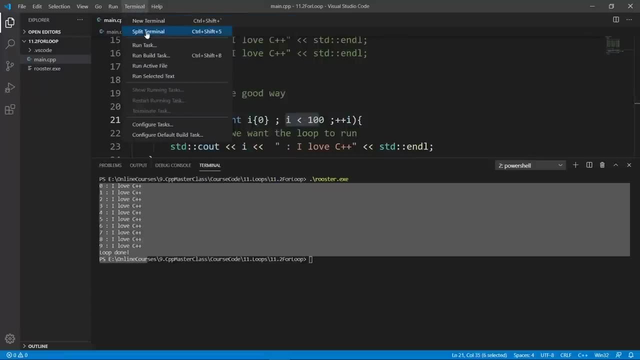 run this. we're going to see the message from 0 all the way to 99, and this is pretty cool. the total is going to be 100 times, so let's build again to show you how cold this is. we're going to run this task. 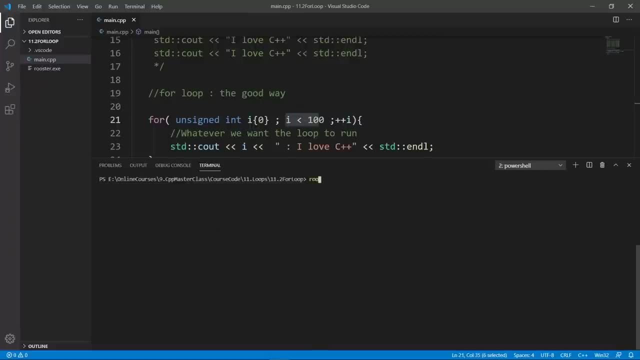 ccc again and we're going to clear run. rooster, prepare to be amazed. run and it's going to run all the way to 99.. we can change this to even 1 000 or even 10 000- why not? we're going to weld. 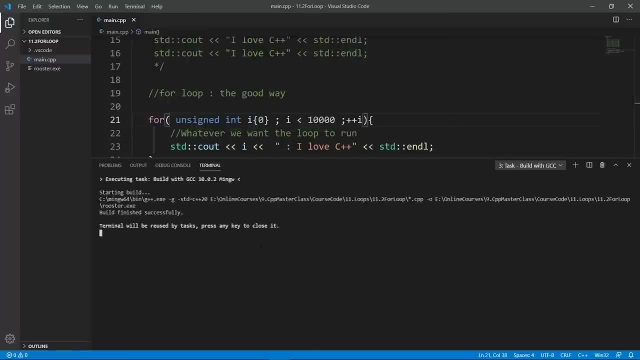 again and we're going to be successful and we're going to clear and run rooster and this is going to go all the way to 10 000 times. we're going to wait for this to get there now: 3 000, 4 000, 5 000, 6. 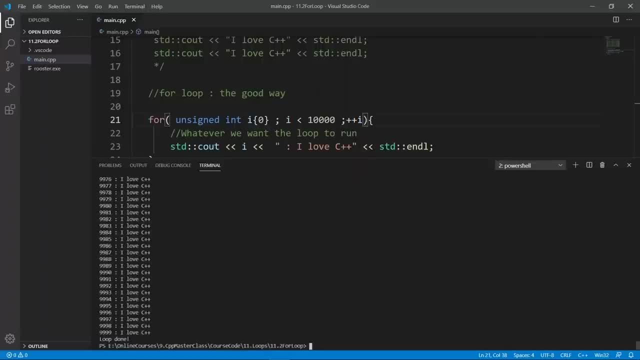 000, 7 000, 8 000, 9 000, 10 000. it's going to go all the way to 9999 and it is going to stop, and the total of times the loop run was from zero all the way to this stopping number here. okay, now we can. 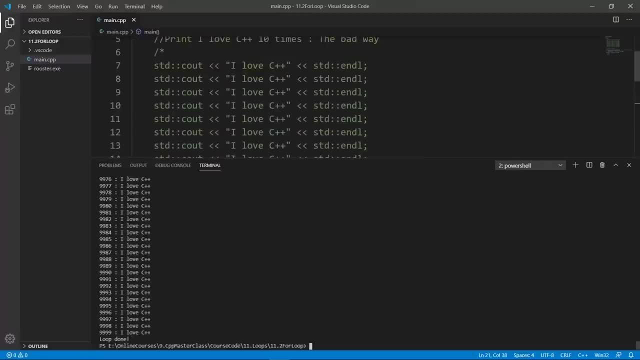 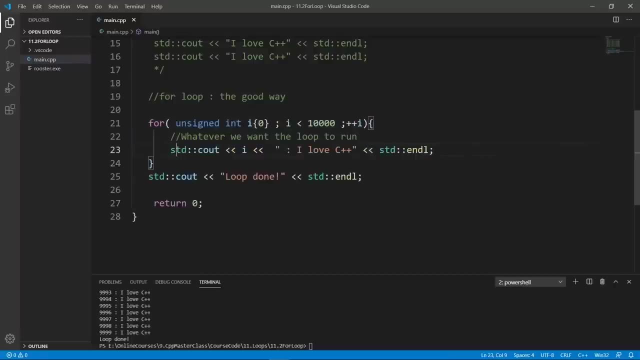 see that our loop is really working. fine. we don't have to do this stdc out statements a crazy amount of times, okay, and the benefit again is that, regardless of the number of times the code here is going to run, our loop is going to stay relatively the same. 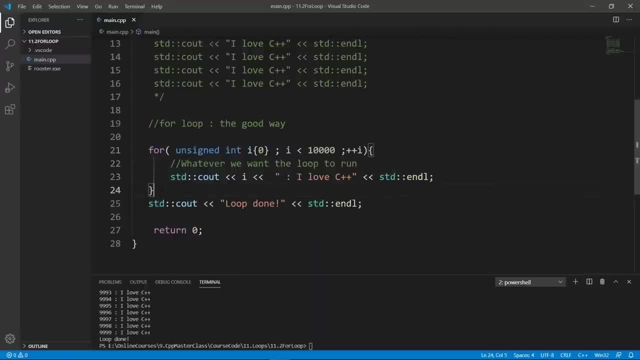 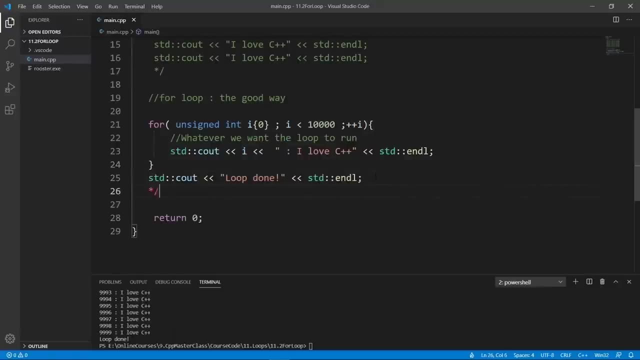 it's just going to be one, two, three, four lines of code, and this is really cool, okay. so i think this now makes it very clear how loops work. so we're going to comment this out and show you another thing, and we're going to show you that you can use size t to actually denote. 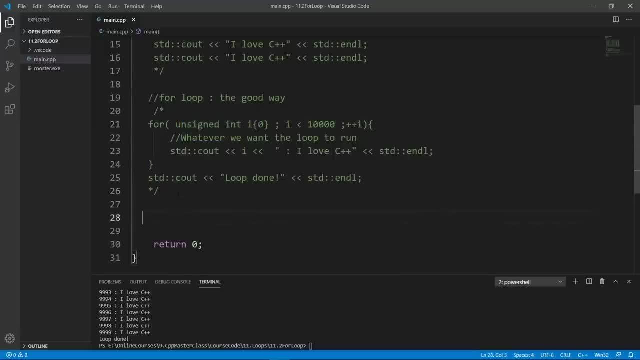 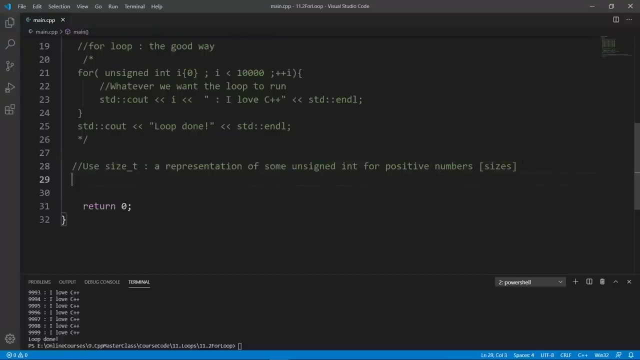 the type of your iterator, and it is easy to do that. so we're going to say, use size t and for us to be able to see all this here, let's hit this file icon here to close this pane, and we're going to have a better chance of seeing our code here. so what we want to do, we're going to declare a loop. 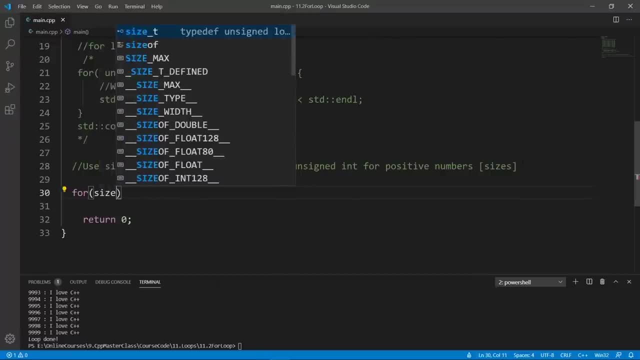 we're going to say four, we're not going to say unsigned, and we're going to say size t, and this is going to be the type of our iterator. we're going to say i, we're going to initialize this with a 0 and we're going to put a semicolon, like we just did. we're going to put in the end test. 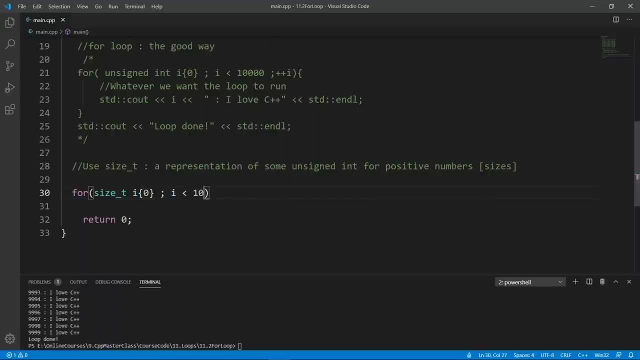 we're going to put in the test. so we're going to say i less than 10, no problem with us. and we are going to increment to put in place our incrementation part. we're going to fall in the loop. we're going to say: stdc out, this is the code we want to run. so we're going to put in our. 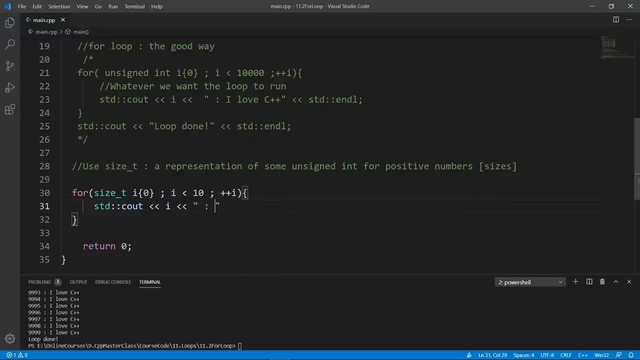 current value for the iterator and we're going to say i love c, plus, plus again. and we're going to put in our new line character and if we build and run this it's going to build and run the same. so let's say loop done here so that we know when it's done, and we're going to build and run. 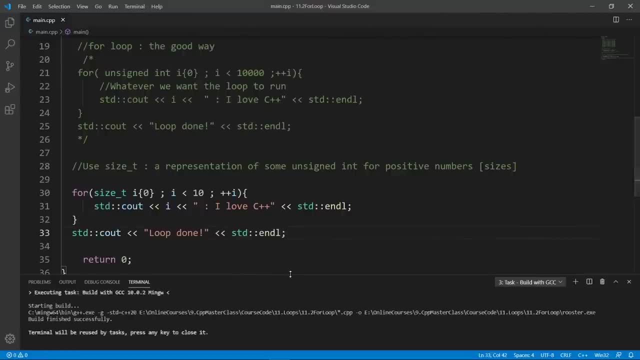 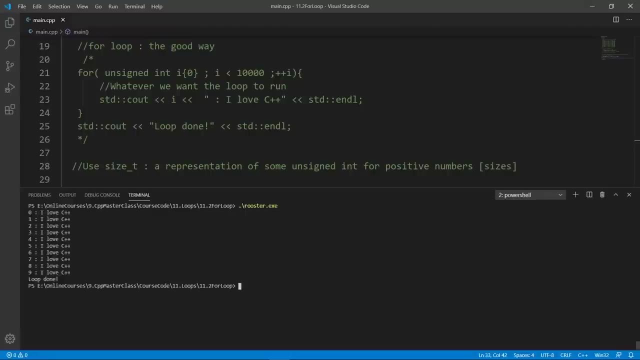 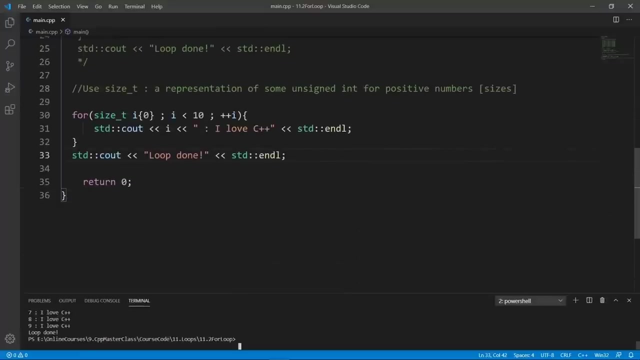 we're going to work with gcc, the world is going to be good, and what we're going to do? we're going to clear and run rooster and this is going to say: i love c plus plus 10 times from zero to nine. again. the message here is that you can use size t to represent the type of your iterators. 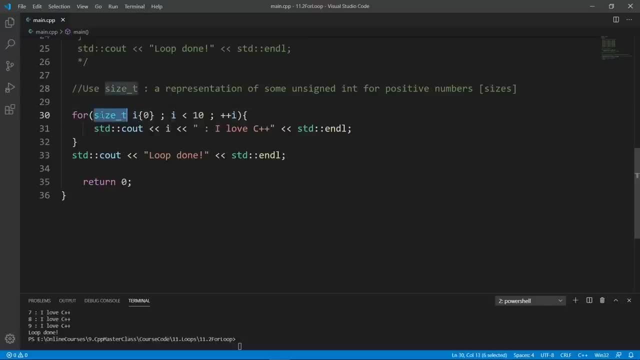 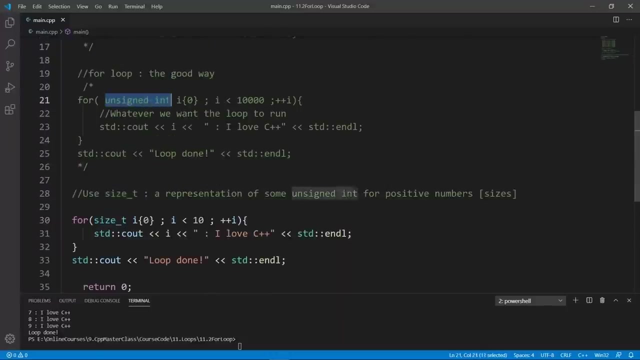 and this is a type that is even used in the c++ standard library. so this is going to be something people expect from your code. if you are representing sizes in code that should be compliant with the c++ standard library, nothing stops you from using unsigned it like we do here, but we're just going to follow the convention from the c++ standard. 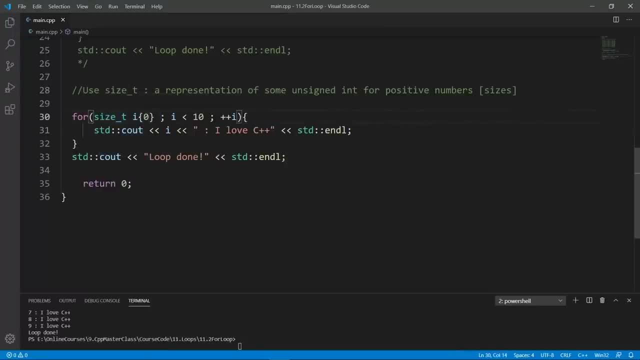 library and use this type here to represent our sizes. and some of you might be wondering: how big is this thing? we have the tools to know how big it is, so let's do that pretty fast. so we're going to go down here and say, sddc out, and we're going to say size, of size t, and we can print this out. 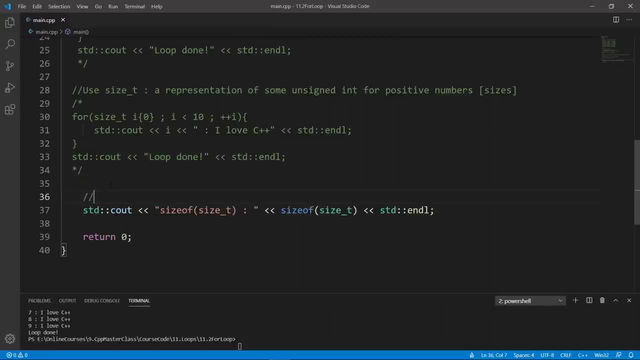 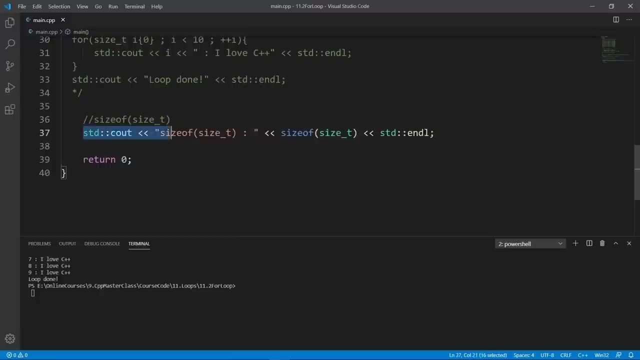 and let's say what we are doing here, so that it is easy to use this code as the reference. and if we print this out, we're going to see the size of this thing on the system where this code here is going to run. so we're going to 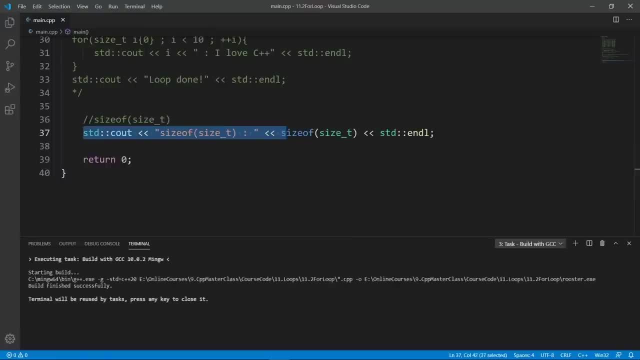 you build with gcc again, the world is going to be good. we're going to go here and clear and run rooster. you're going to see that it is eight bytes on my system, so you're going to have quite a huge range of numbers you can put in here, because this is going to only be positive. okay, if you try to put. 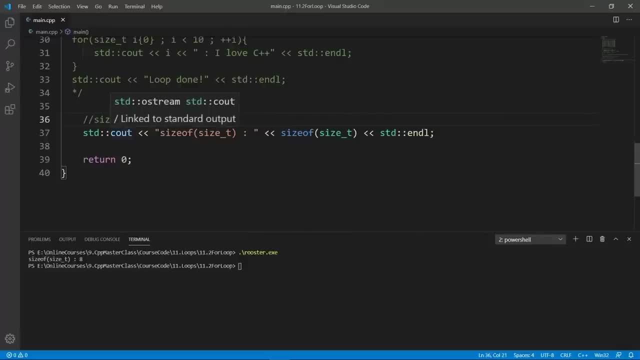 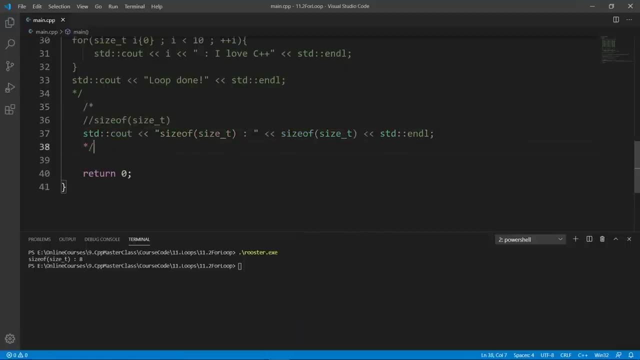 keep learning more things about for loops. okay, the next thing i really want you to focus on and learn is the scope of the iterator, and we're going to grab our code again here so that we can use this as a learning tool. so we're going to go down here and put that in and what we're going to have. 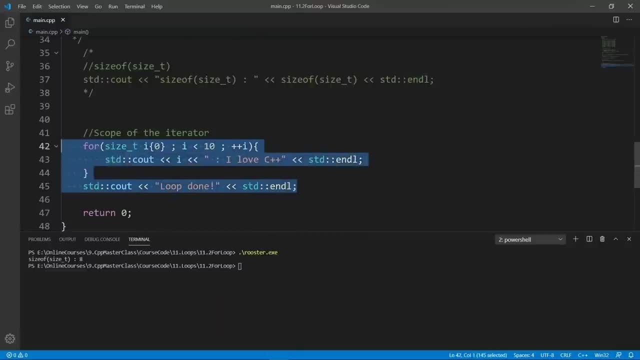 let's move this a little bit to the right. i think we can do something like this: i am going to select the entire thing here and hit tab, and it is going to be the code that we're going to use for this to be aligned with whatever we have here. okay, so we have our loop. it is going to run 10 times, it's. 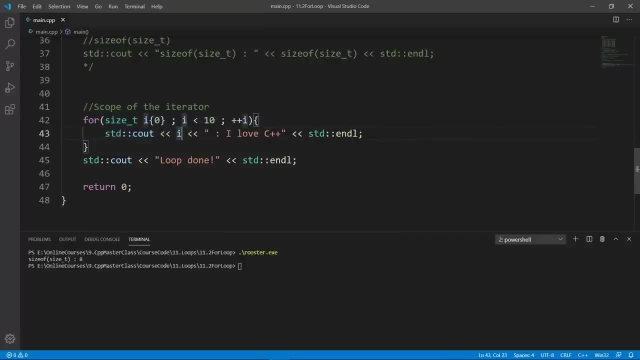 going to print. i love c++ from zero to nine. but what is the scope of this? i think here, and the fact is it is scoped inside this loop. here you might have guessed that if you try to use it outside the loop you're going to get a compiler error because it is only usable inside. 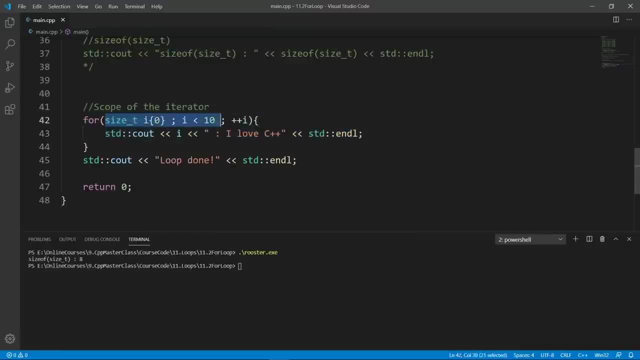 the body of the loop. you can also use it inside the controller if you want to use it inside the control part of the loop here. but you can't use it outside the loop. so if you try to print i here, for example, you're going to get a compiler error. so let's try and do that and show you how wrong. 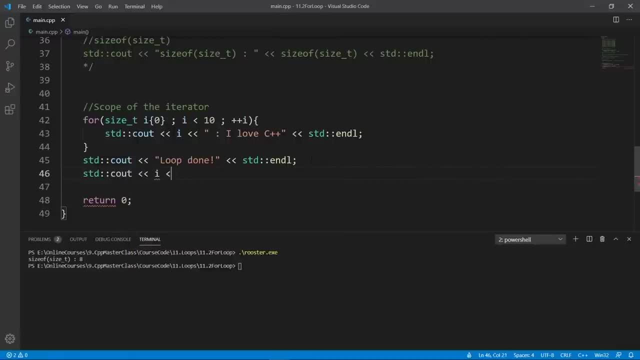 this can be so if we try to print- i here, let's say i to make it clear what we want to print- if we try to do this, we're going to get a compiler error because i is not in scope, it is only in scope inside these curly braces that show the body part of our loop. okay, visual studio code. 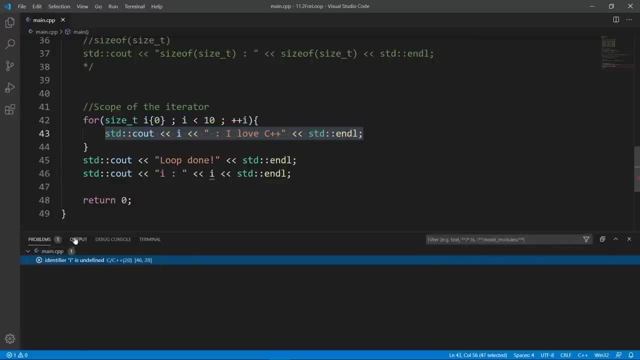 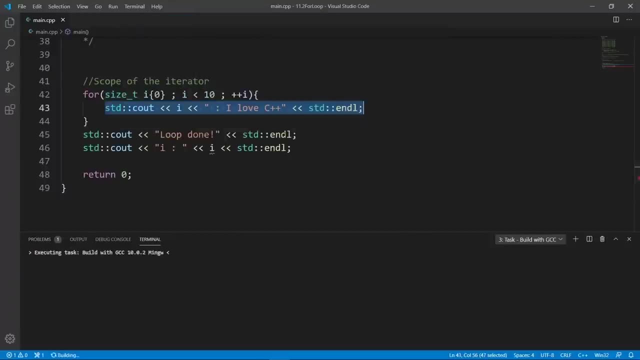 is showing the problem here. it's saying: i is undefined here, so you shouldn't really do this. but if we move on and ignore the message from visual studio code and compile, we're going to get a compiler error and it's going to say: i don't know what you're doing here. i was not declared in. 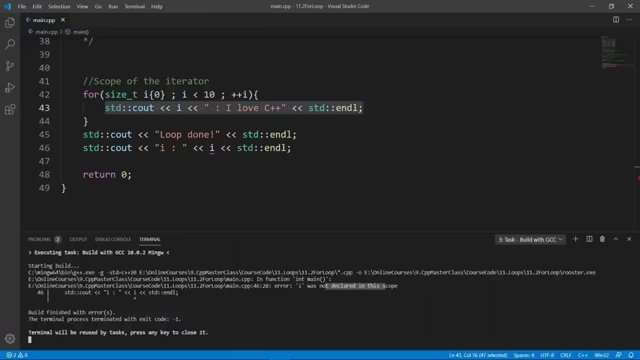 this scope where you are using it, and i think it's even going to give me a line number. it's going to tell me 46. that's where you are doing something wrong and if we go in our code, we're going to see that this is the line where we are making the mistake. so i is not in scope here. we're going to comment. 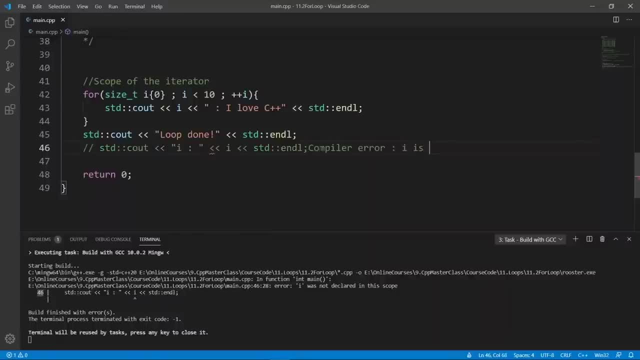 this out and say: compiler error, i is not in scope. that's what you're going to get if you try to do this, and the main message is that if you declare your loop like this, i is only going to be scoped in the body of the loop and that's the only place where you can mention its name and use. 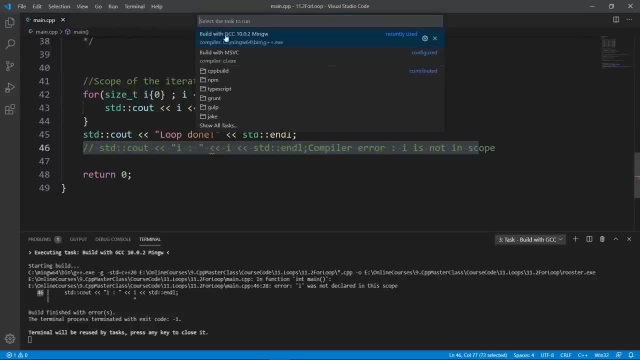 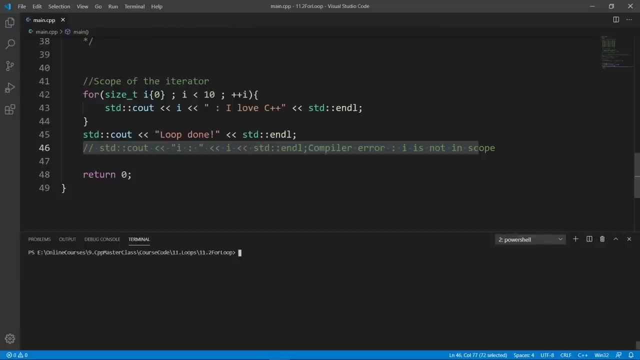 it. if we comment this out and weld again, the compiler error is going to go away. you're going to see that the world is good. let's clear so that our output here is good. we're going to build again and show you that the world is good and, uh, this is really cool. world finished successfully, okay. 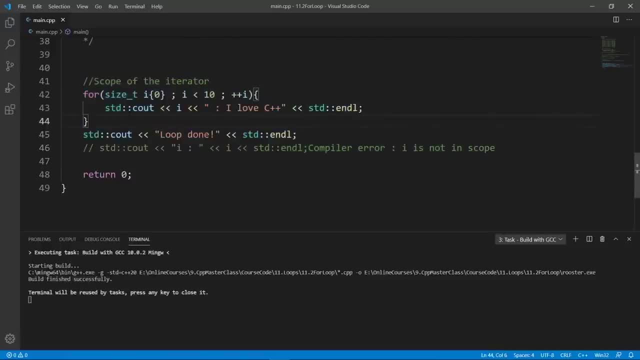 this is one way we can set up our loop, but there is a way we can make our iterator usable outside the body of the loop, and we're going to show you how you can do that next. so let's comment this out and go down again, and we're going to grab the code because we don't want to type all this again. 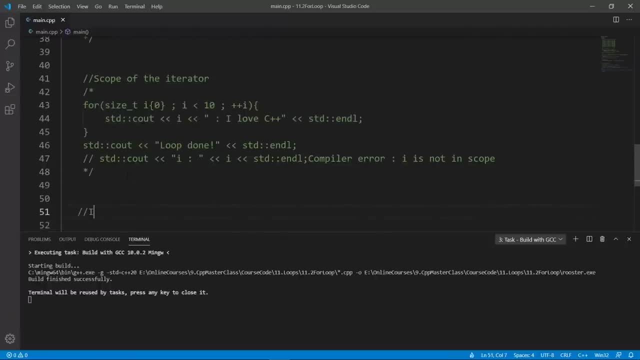 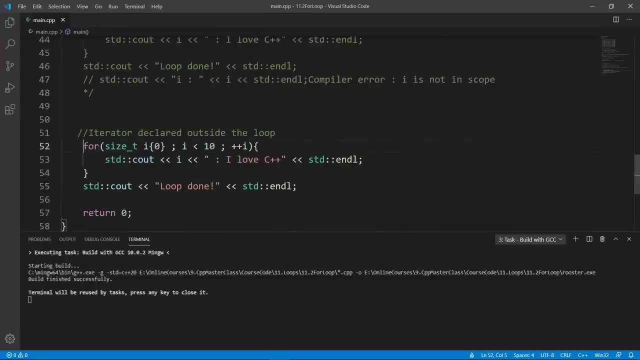 and we're going to say: iterator declared outside the loop. we're going to go down and put in our code and we're going to align this nicely and we're going to take the iterator and declare it on the outside of the loop. so we're going to say size t and we're going to say i and initialize this to 0. 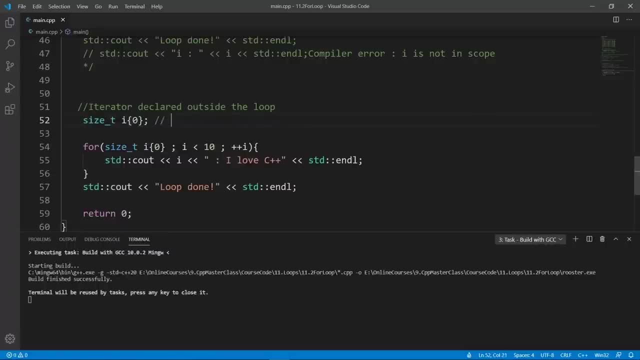 and we're going to say this very clearly: iterator defined outside. and we're going to say in our declaration: part of the iterator. we're going to just say i, and this is going to work pretty fine. if we weld this, you're going to see that the world is good and if 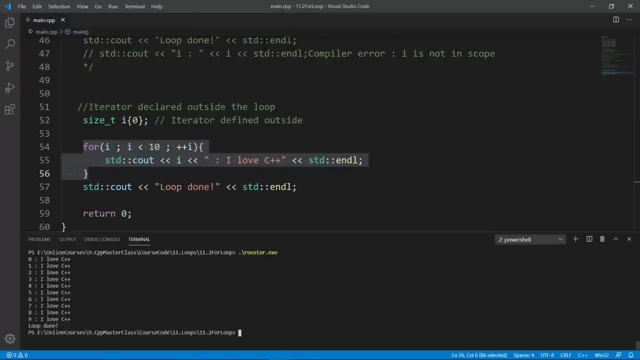 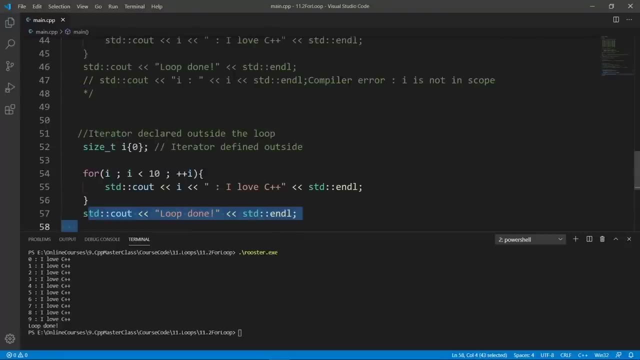 we run this, it's going to do the same thing it's been doing. it's going to print i love c plus plus times and if you want, i usable on the outside of the loop. now you can use it. we can grab the code here that was failing in the last run over our code and put that out here and we're going to. 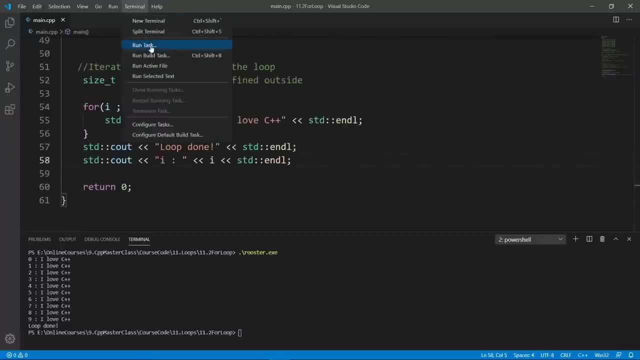 align this a little bit and if we compile this, the build is going to be good. and if we try to run rooster, we're going to see i love c plus plus 10 times. we're going to say loop done and we're going to print the value of i. and you see that if we do things like that, we're going to see a loop done and we're going to print the value of. the later we're going to print the value of i and you see that if you- I don't want to say your magic, though we see teams don't fool around. I'm not sure that the loop Kenyaject the ilma robot, but let me read this- should say: do thing like that information and- and I'll be happy if w complain e e without that. 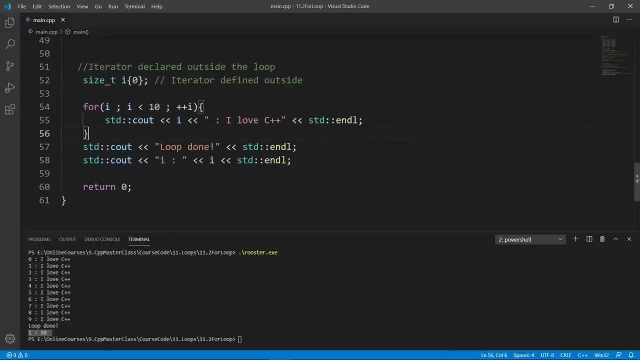 this i is going to be usable on the outside of the loop body, and sometimes these may come in handy, depending on the logic of the application that you are designing. just know that this is something you can do in your loops. okay, you can go even crazier and leave out this. iterator declaration part. 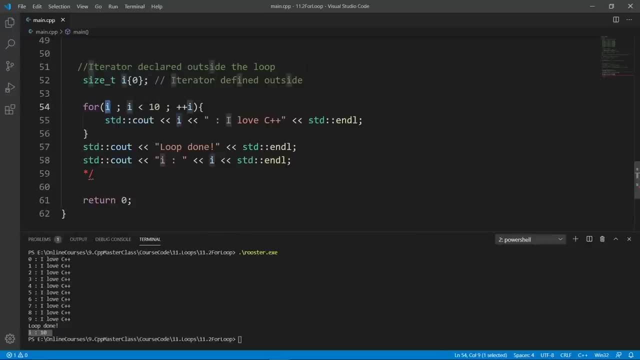 in your loop altogether. so you can remove that and we're going to show you how you can do that in a minute. so let's comment this out. i don't want to remove code because i want you to have this as a reference if you need to look at this later. so we're going to say: leave out and what. 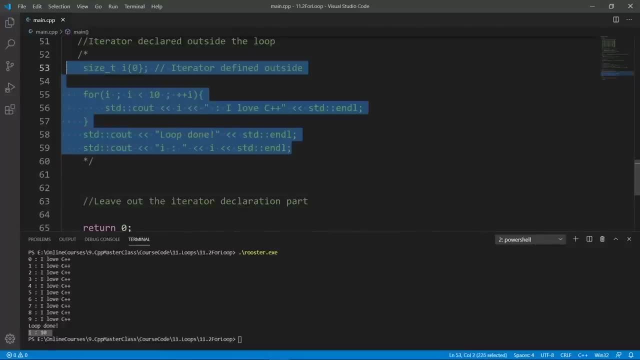 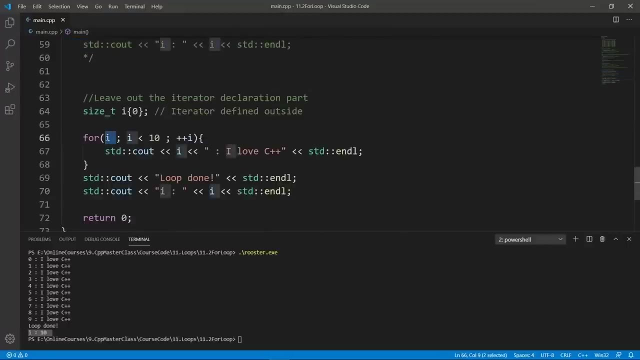 you can do is grab the code we had before. we're going to grab it and we're going to paste that in here, and what we're going to do is take out this i- this can work and you may see code like this out there in the wild. so we're going to run the task to build with gcc. the build is going to be. 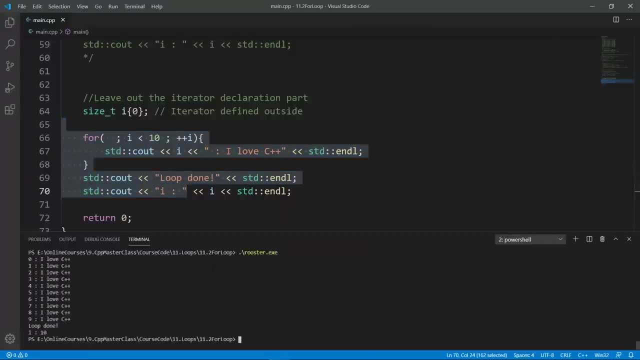 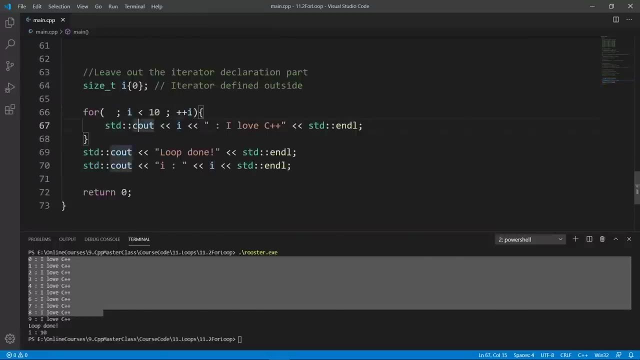 be a little bit more complicated. so we're going to run the task to build with gcc. the build is going to be good, and we're going to clear and run rooster and it's going to do exactly the same thing. so this is one way you can set up your loops. okay, the last thing we need to see about loops is that this: 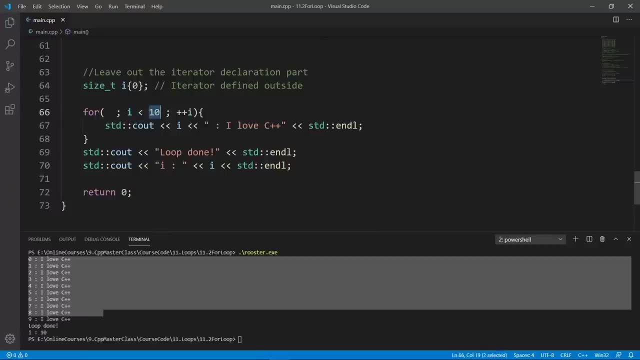 test here is using a hard-coded value, and if we needed to change this loop to run, for example, for a thousand times, we would need to manually hunt for this line of code, change this, and this is really not good design. so what is recommended is to store this value in a variable. 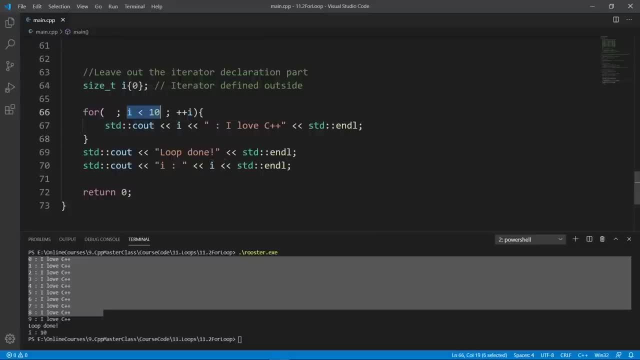 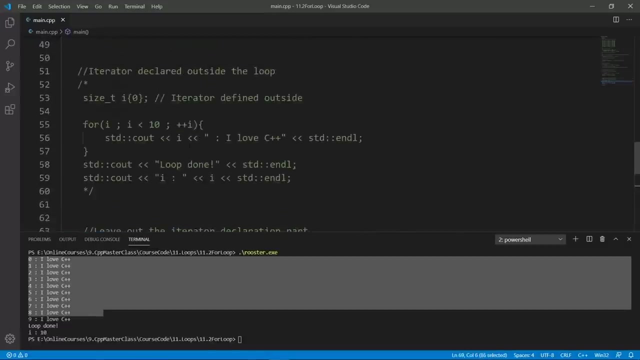 and test against that variable name. instead, let's comment this out and show you that. so we're going to comment this out and go down and copy this entire thing. i don't think i want to do my loops like this, because this is really unintuitive most times. so i am going to declare my iterator inside. 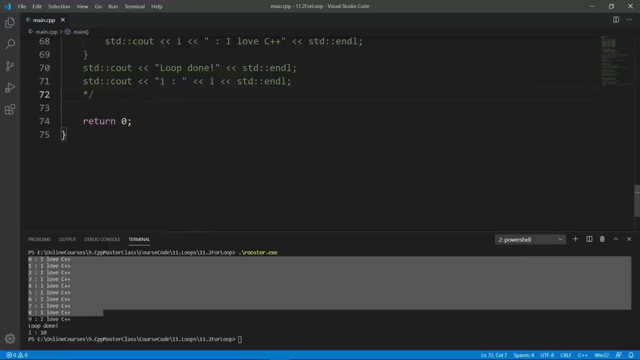 and i'm going to copy the code that does that. here we're going to go down and say: don't hard code values. okay, we're going to say that it's really bad and we're going to go down and show you a better way to do. 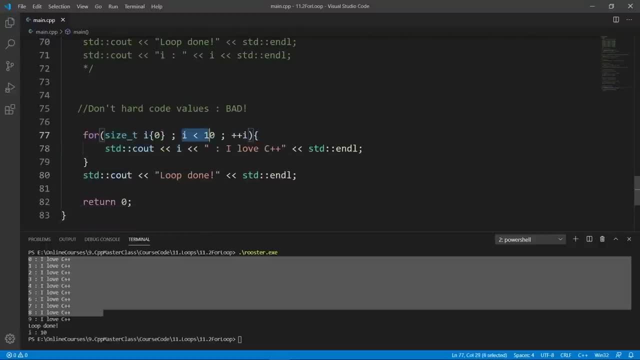 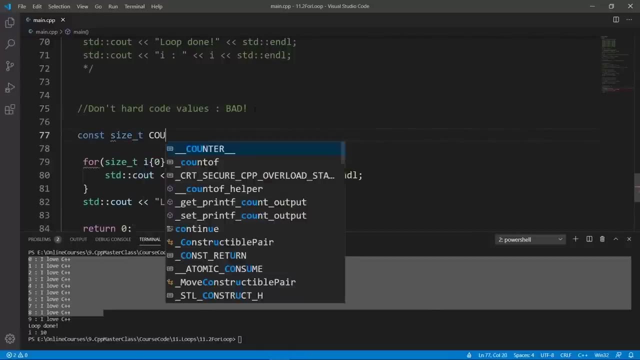 things. and again, right now we are hard coding in this value, but we can say cost size t and we can call this value count, for example, and we can initialize it with whatever we want. in this case, we want to control our loop to run 10 times. 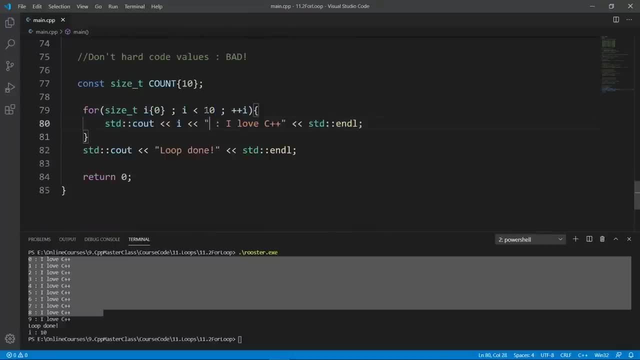 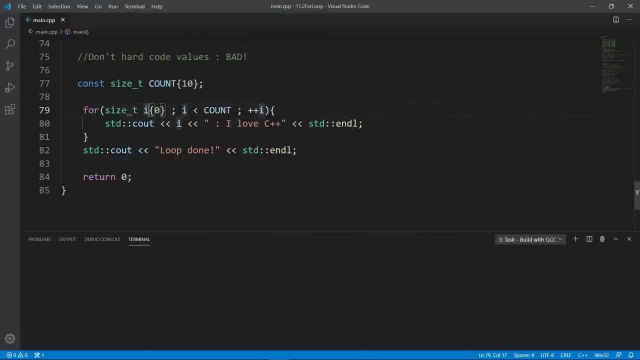 so we're going to put in a 10 and instead of hard coding and this 10, we're going to say count, okay, and if we build and run it, the loop is going to do exactly the same thing. it's going to print: i love c plus plus 10 times. so let's do that and run rooster. it's going to do the same thing, but 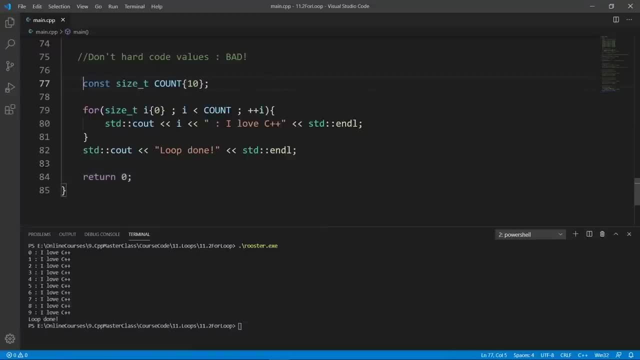 now we have one point of control: if we want this to run for, let's say, 100 times, we can change the count value to 100 times, and if we both, again that's how many times the loop is going to run, and this is much cleaner. so i do recommend you to store a which runs this information as 100 times. 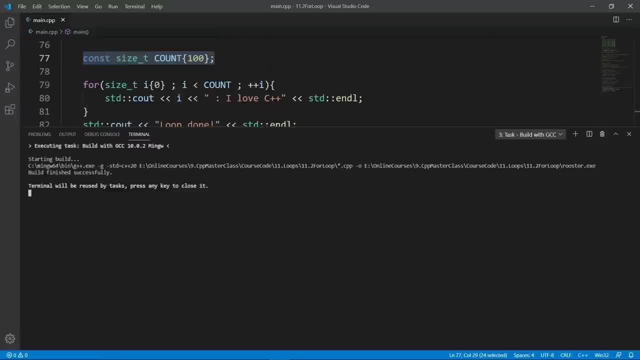 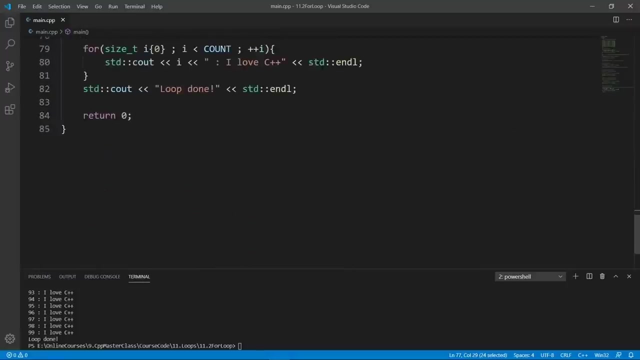 the values you use in your loops, in variables like this, and it's going to make your code look better. so it's going to run 100 times, and this is exactly what we want. this is really all we set out to do in this lecture. i hope you found it interesting. i am sorry that this lecture turned. 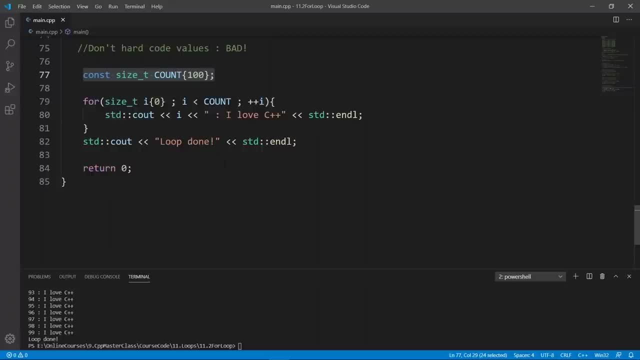 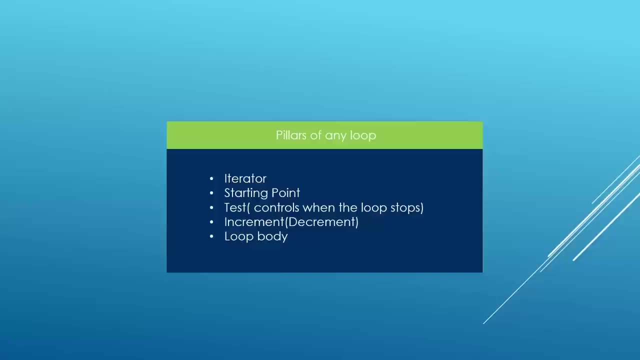 out lengthy because we had a lot of things to talk about, but now i hope you really know a lot of things about ways you can use your full loops to make them do things. and again, many loops that we're going to use in our c++ code are going to have five parts. we're going to have an iterator. 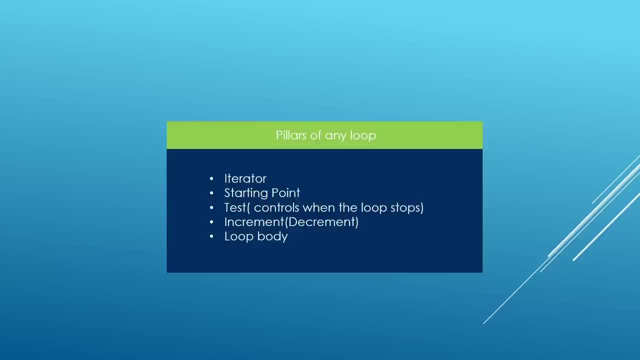 which is going to be a variable we use to manipulate how our loop moves forward and does things. the starting point is going to be where the loop is going to start. we're going to have a test in place which is going to control when the loop ends, and we're going to have the end. 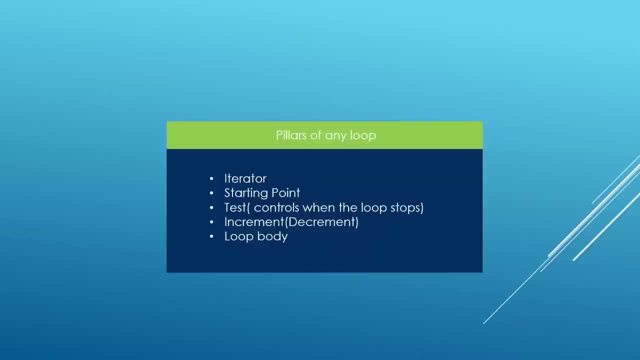 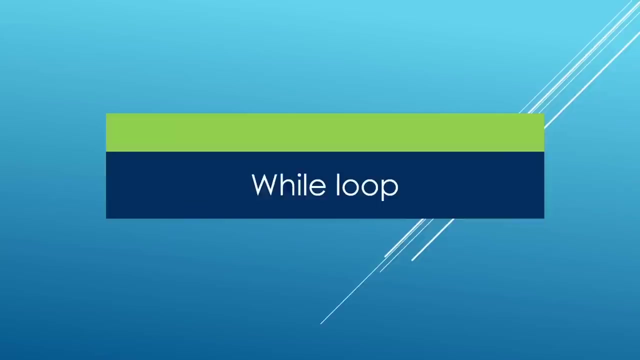 point encoded in that test. we're going to have the incrementation part of the loop, which is going to control how our loop moves forward, and we are going to set up a pair of curly braces that are going to contain the body of our loop. in this lecture we're going to learn about while 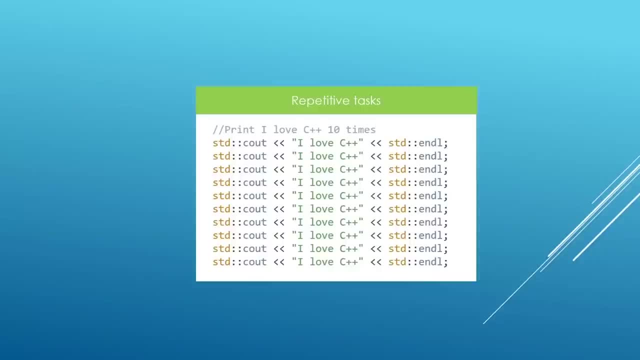 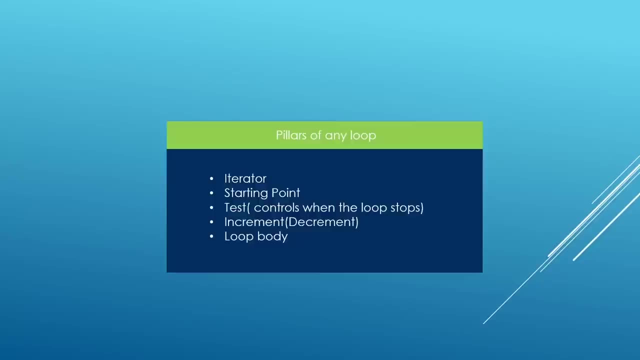 loops, and this is another construct we have in the c++ programming language to allow us to do repetitive tasks. the syntax for a while loop looks like this: we have five parts in our loop. we have the iterator, the starting point, the test, the incrementation and the loop. 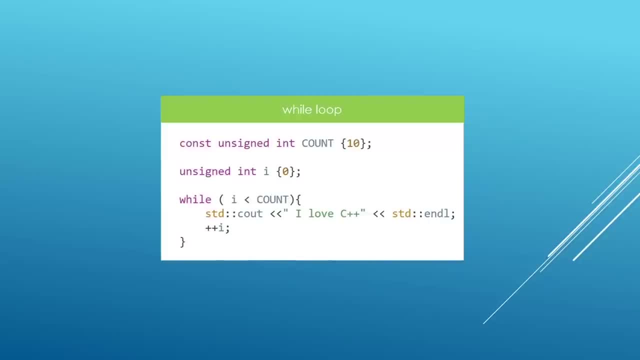 body. it's just going to be set up differently for while loops. the iterator is declared on the outside and you see, here we have unsigned and i, which is exactly the same type of iterator we've used in the last lecture, but know that you can also use size t here i am just using 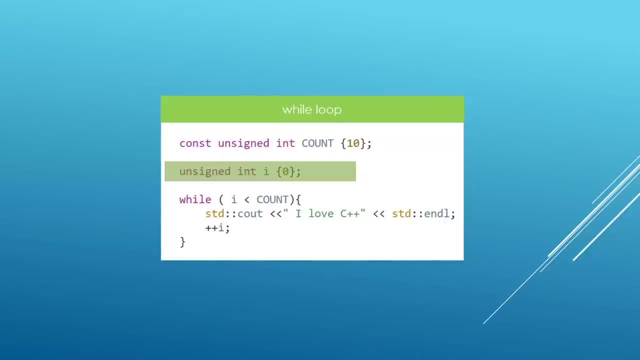 unsigned and, for this case, after you have your iterator declared, you're going to fall to this part here and say, while open, a set of parentheses and inside you're going to put in your curly braces and inside them you're going to put the body of your loop and you're going to do: 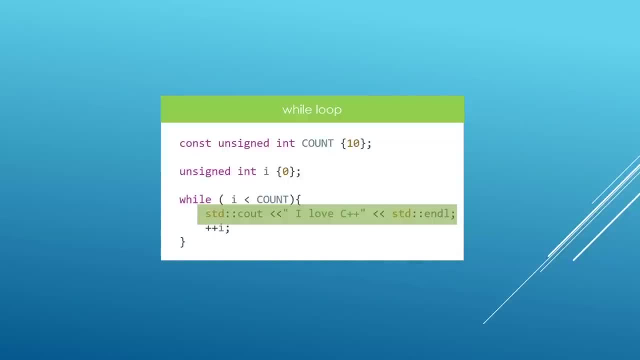 whatever it is you want to do in the loop, in there and after your code to do whatever it is you want to do is execute it. you're going to put in your incrementation part after your code and that's what we have here and this is the setup we're going to be using for our while loops. again, we 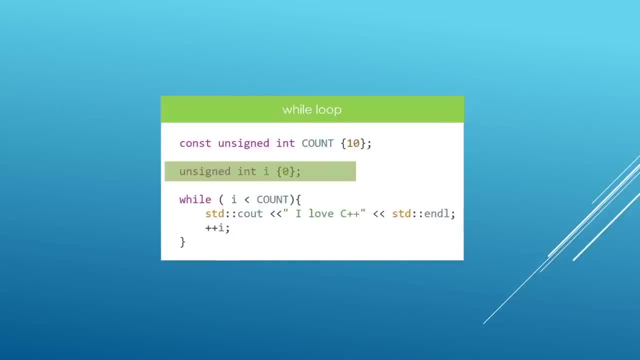 have the iterator declared on the outside and we're going to put in the body of your loop and the outside and we can initialize it with whatever it is we want to start with. then we're going to put in our test. it's going to be within this parenthesis and after that we're going to set up. 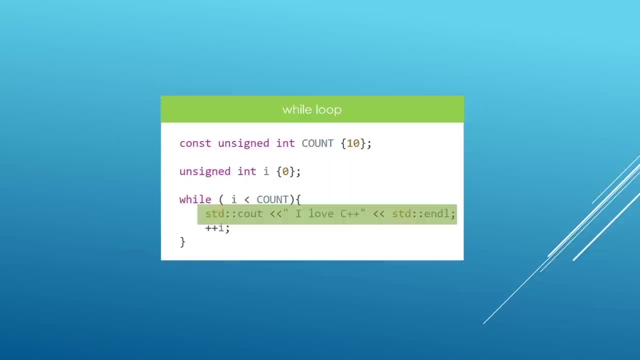 a pair of curly braces and inside them we're going to put whatever code we want to run in the loop and then we're going to follow that with our incrementation part and if we try to run this, we're going to run this line, we're going to declare the iterator i and it's going to start. 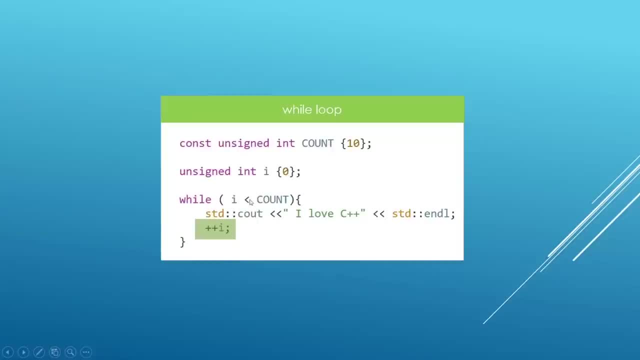 with zero. so the test is going to run and zero is less than ten and we're going to succeed and we're going to run the body here. we're going to say i love c plus plus and after that we're going to run the incrementation part. 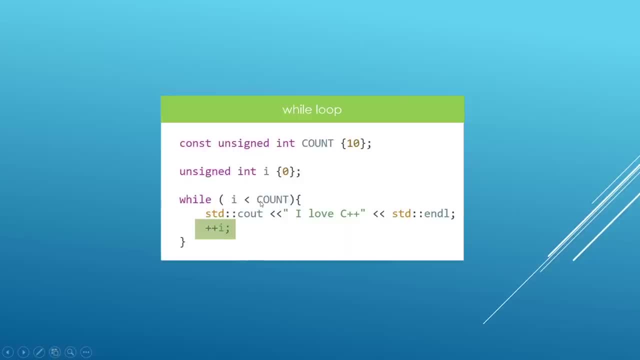 i is going to become one. we're going to run the test again. so one is less than ten. we're going to succeed. we're going to fall in print: i love c plus plus. we're going to increment again. then we're going to have a two in i here. we're going to run the test again. we're going to say is two. 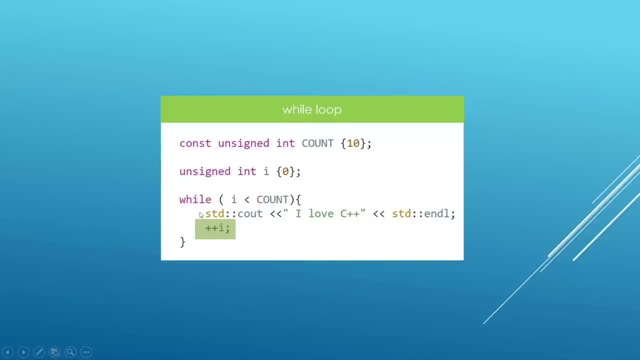 less than ten. that's going to be true. so we're going to run the test again and we're going to be successful. we're going to fall in the body of the loop. we're going to increment and get a three. we're going to test against our three value three is less than ten. we're going to succeed. we're. 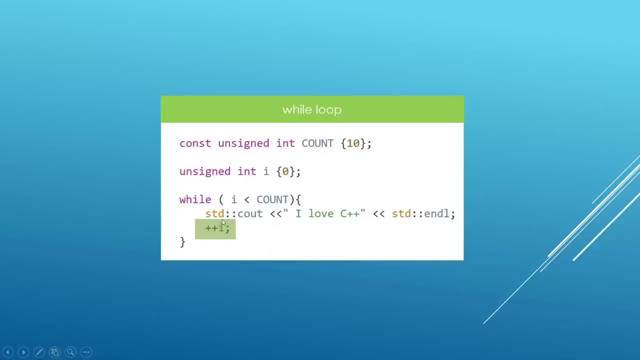 going to print: i love c plus plus. we're going to increment again, we're going to test again and we're going to say: is four less than count or ten, we're going to be successful and we're going to keep running until we increment and get a nine. once we get a nine, we're going to run the test. 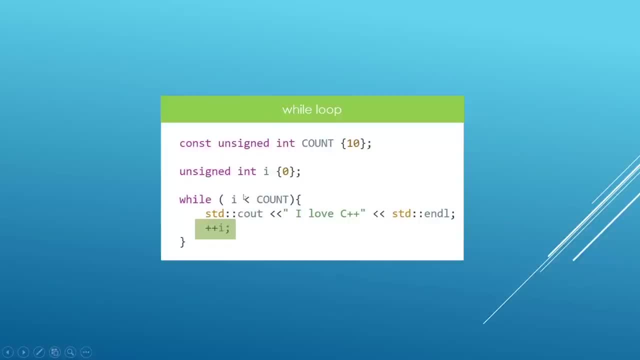 again and we're going to say: is nine less than ten, that's going to be successful. so we're going to fall inside print: i love c plus plus. we're going to increment and get a 10 and if we run the test again, we're going to say: is 10 less than 10, that's going to fail and we are going to fall on. 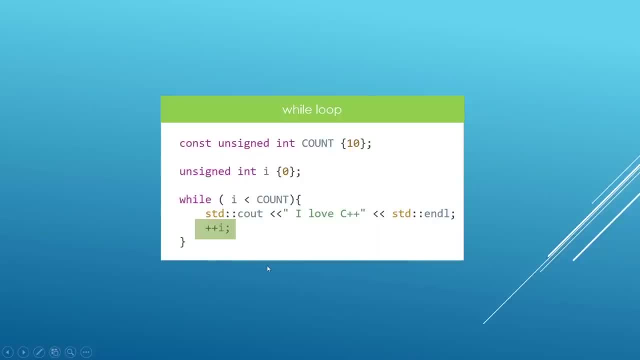 the outside of the loop and we're going to run whatever code is on the outside here. this is really how a while loop works and i hope you can see the similarities between the four loop we have seen. it is really the same thing. we just have different syntaxes to do these things. okay, if you look at these things we really have. 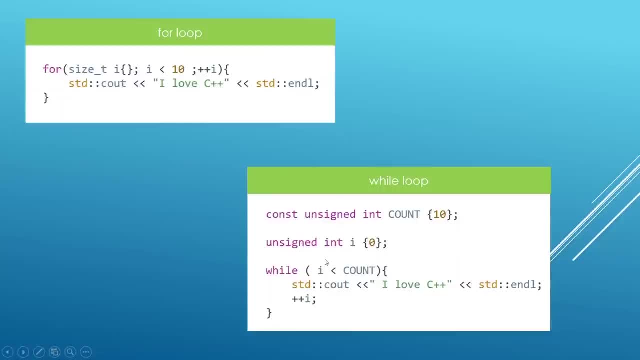 the same pieces of information. it is just different syntaxes that c plus plus provides to do the same things and sometimes you're going to find it convenient to use while loops and sometimes you're going to find it convenient to use for loops and you're going to have to decide what. 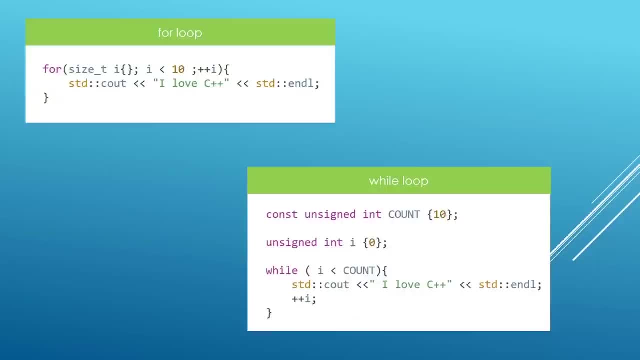 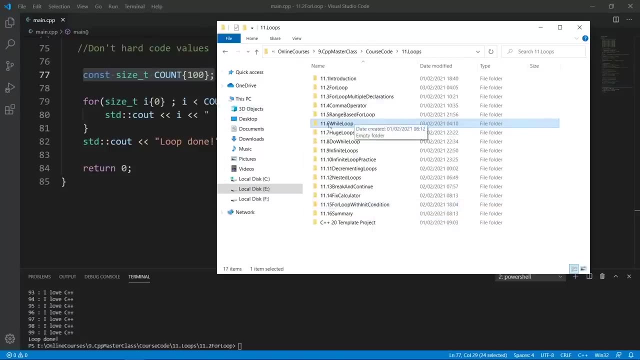 works better for whatever it is you are working on. for now, we're going to head over to visual studio code and try this out. okay, here we are in visual studio code and we're going to run studio code. the current project is while loop. we're going to grab our template files and we're 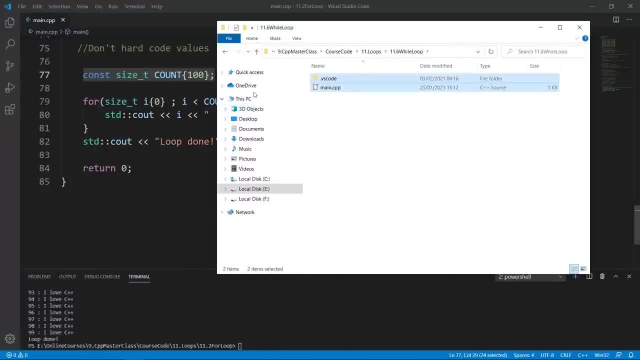 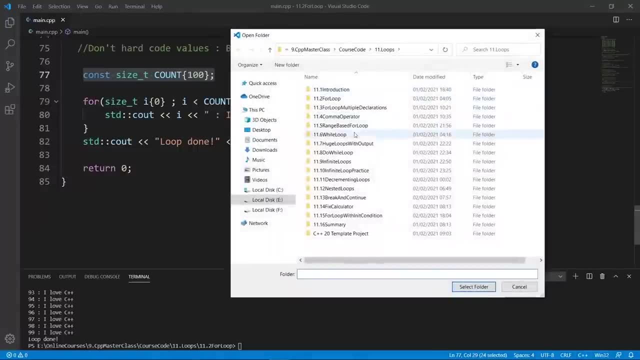 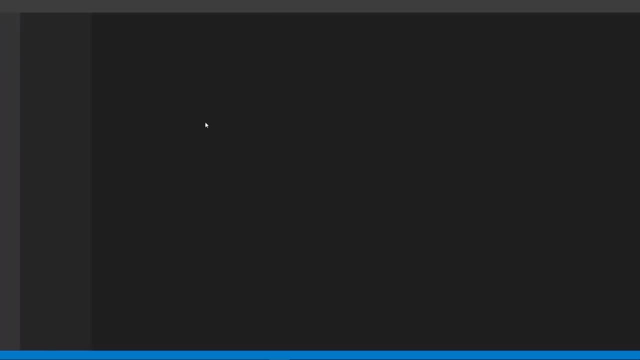 going to go in our project and put those in and we're going to open this in visual studio code, so let's do that. we're going to open the folder and we're going to work on while loop here. we are going to open our main cpp file pretty quick and we're going to get rid of this and what we're. 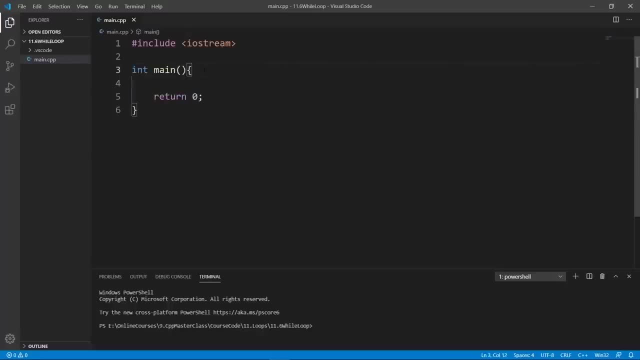 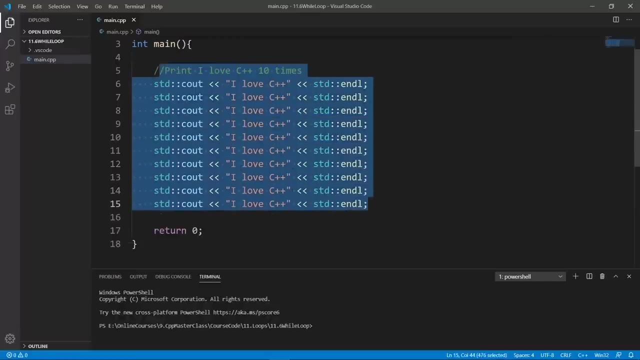 going to do is remove what we don't need and again we're going to show you the bad way to do things. want to do this manually. we want to print: i love c plus plus 10 times. so we're going to build, let's bring up a new terminal so that we can use this when we run things and we are going to world with. 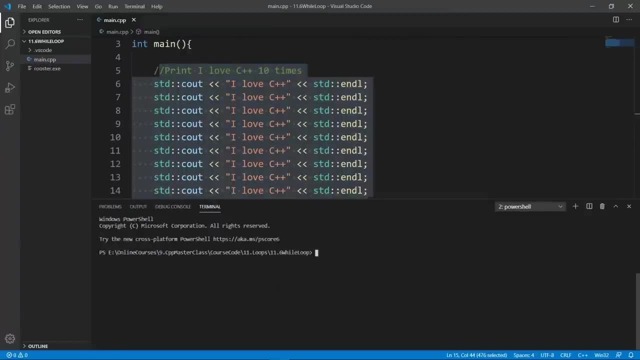 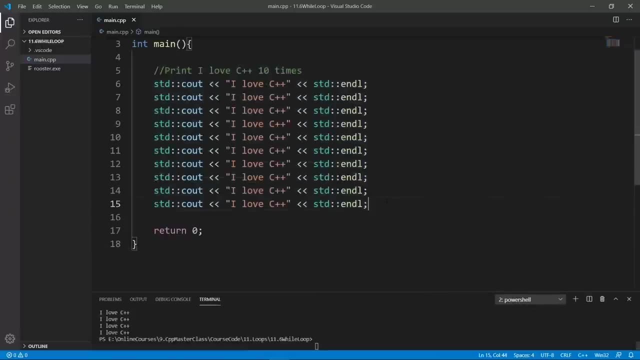 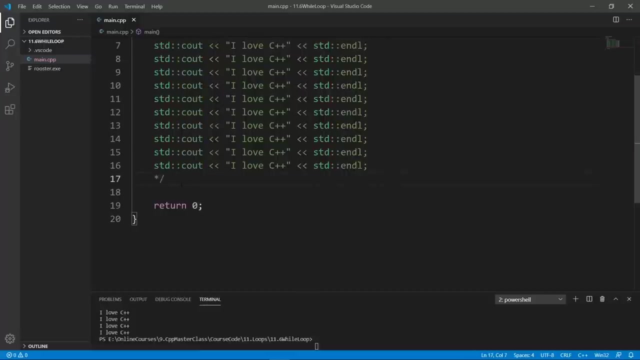 gcc. let's do that pretty quick. the world is good. so we can clear and run rooster and we're going to have i love c plus plus printed out 10 times. so what we can do is comment this out and use a while loop, like we want to do in this lecture here and as we have seen with the slides. 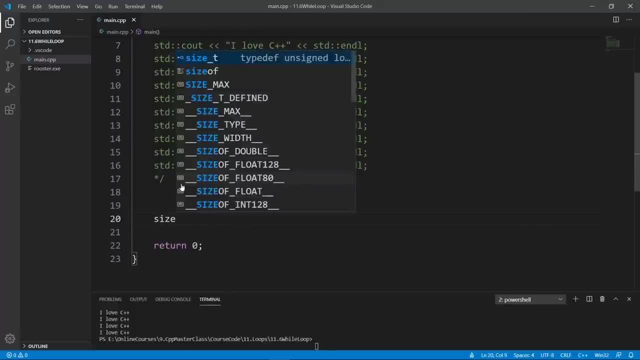 the first thing we need to do is declare our iterator on the outside. so we're going to say size ti, we're going to initialize this with a 0 and that's going to be our iterator declaration. and we're going to say: while i is less than the value where we want to stop, and again we don't. 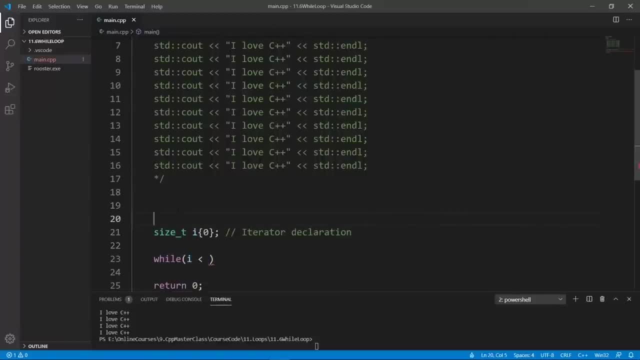 want to hard code these values in. so what we're going to say is really const size t, and we're going to call this count and make it uppercase. this is a convention we use to declare constants in c plus plus, but you don't have to make them uppercase. it is just a convention. 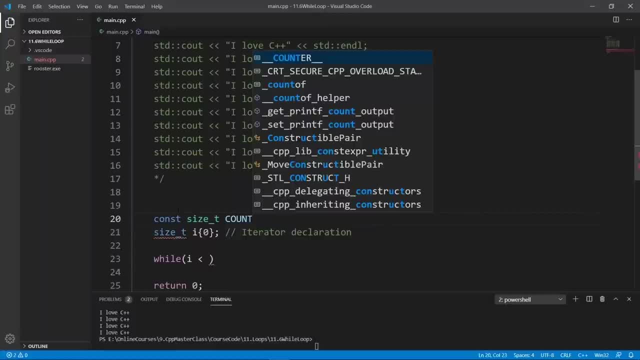 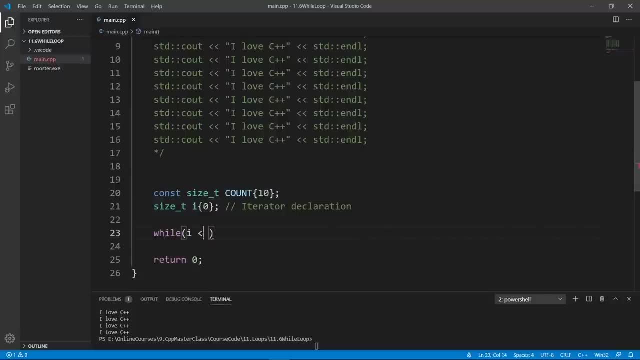 that is going to make your code easier to read for other people. so we're going to put a tan in here because we want our loop to run 10 times and we're going to say why i is less than count. and we're going to set up a pair of curly braces and they are going to delimitate these. 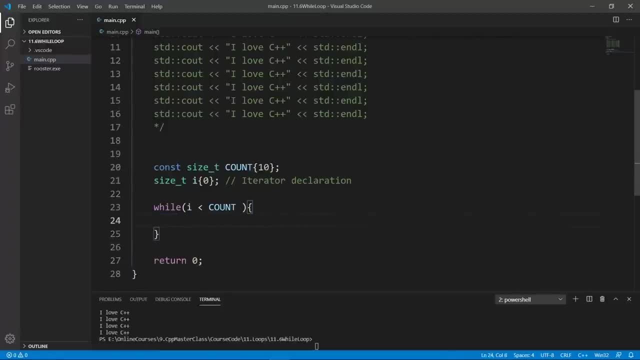 start and the end of the body of our loop. here and inside we're going to put in whatever code we want the loop to run multiple times and the code is now very familiar. we're going to say sddc out and we're going to print the current iteration and we're going to say: i love c plus plus. 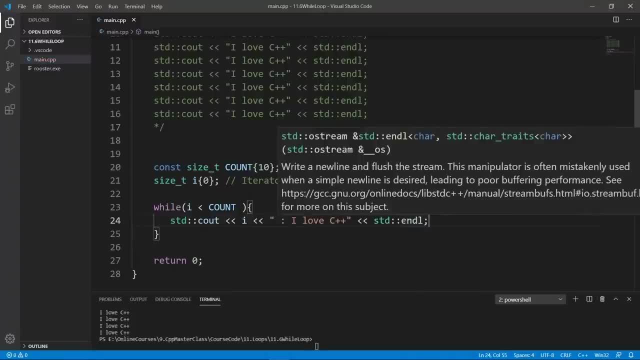 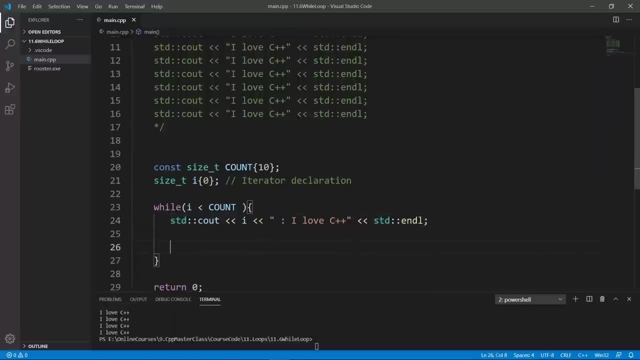 std endl for our new line character and after that we will need to put in our own incrementation part. if you forget that, you're going to get something really bad happen. but then we're really going to look at that later in the chapter, but for now remember to put the 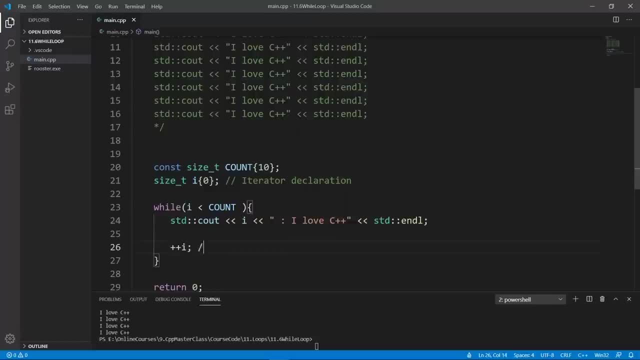 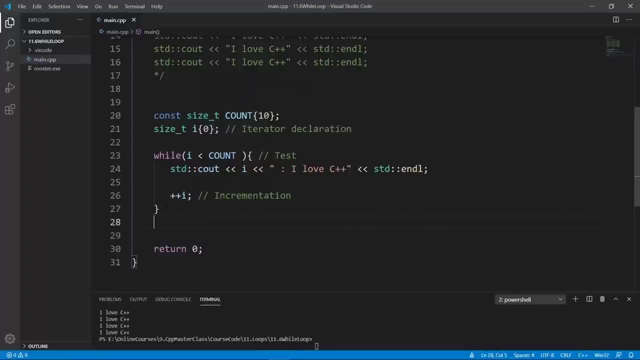 implementation part, and we're going to say plus, plus i- this is really easy and we're going to say that this is the test and this is going to do what we want. but let's go down here and say that loop is done when it is done, so we're going to say loop done and we're going to say std endl. 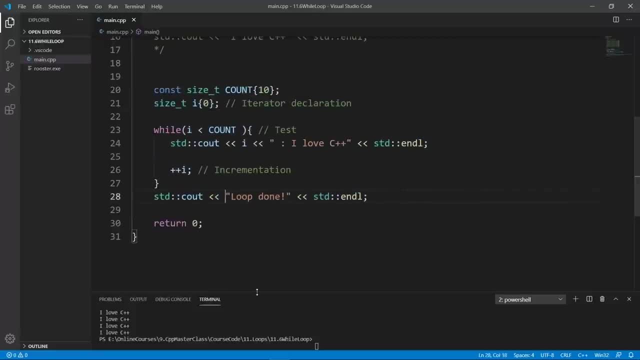 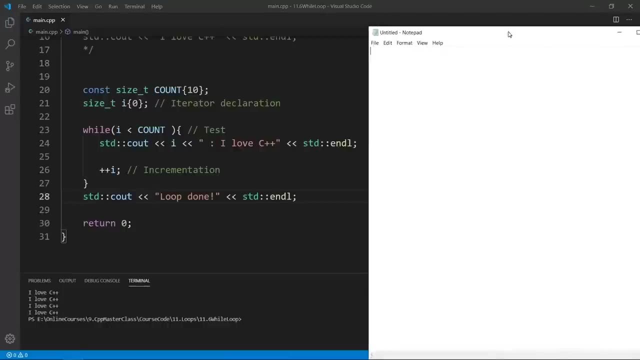 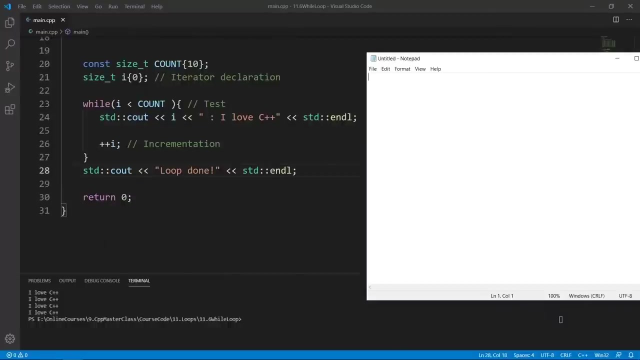 this. we're going to go through it and see how it is going to work. so let's click on this file icon here to close this pane so that we have some breathing room. i am going to open a notepad file we're going to use to see these things really happen when this loop runs. we're going to 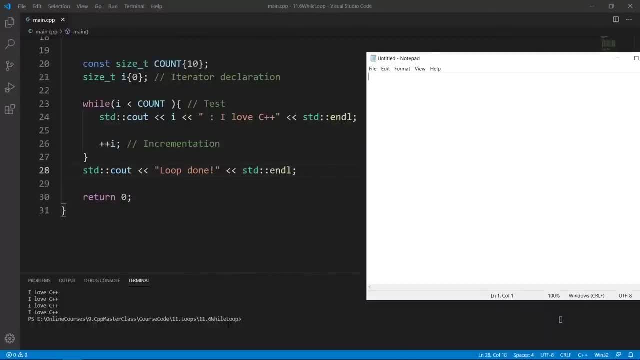 initialize the iterator here. what we're going to do is put in a 0 and we are going to run the test to see if 0 is less than 10 and the test is going to be successful. so we are going to fall in here and say 0, i love c plus plus. so let's say that here to make this super clear inside the loop. 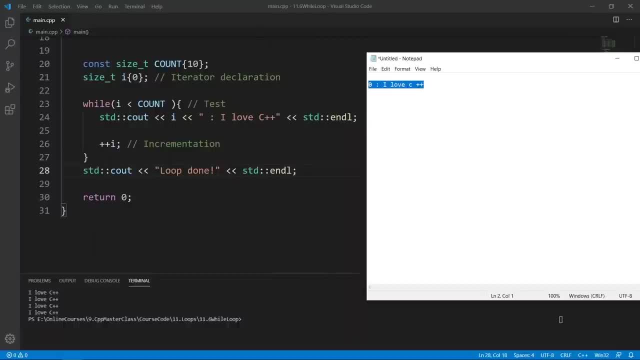 we're going to print this message: 0 i love c plus plus, and after we execute this line, we're going to increment. i is going to become 1. we're going to go up again and run the test and we're going to say: is 1 less than count or is 1 less than 10.. the test is: 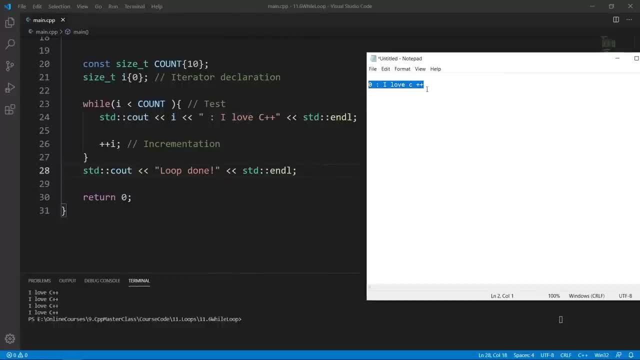 going to be successful. we're going to run inside the loop and we're going to print 1. i love c plus plus. that's what we're going to do here, so let's do that. and after we do that, we're going to run our incrementation part again. i is going to become 2. we are going to run the test. we're going to say: 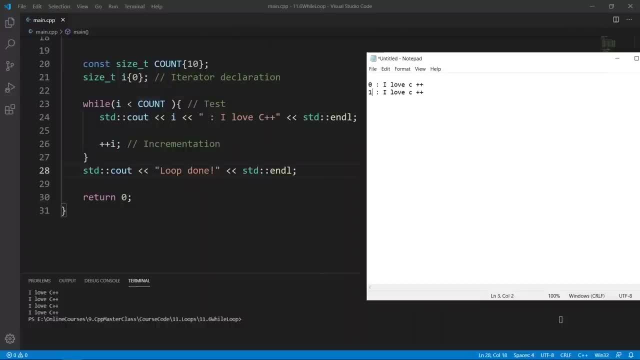 is 2 less than 10. that's going to be true, of course, and we're going to fall in the body again and say, 2 i love c, plus, plus. so let's say that we're going to implement and we're going to get a. 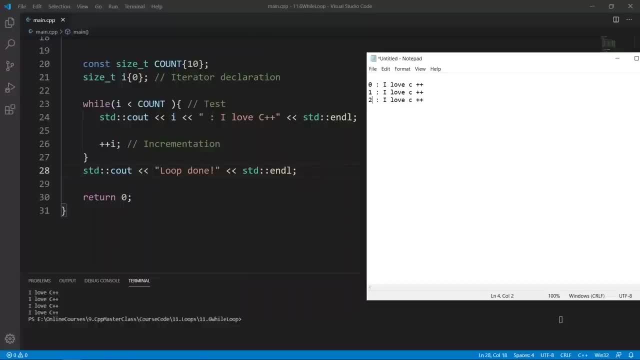 3. going to run the test again. the test is going to be successful because 3 is less than 10. we are going to fall in here and say, 3, i love c plus plus. okay, so we can really follow this and we are going. 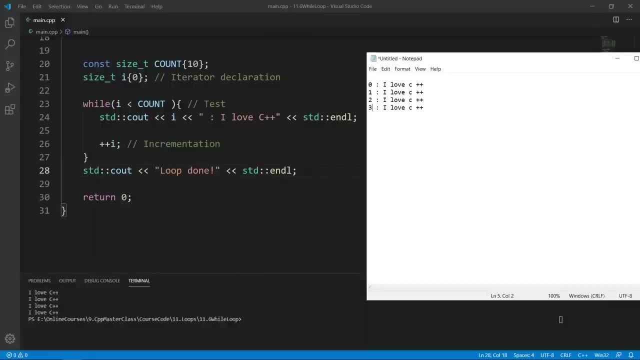 to increment to get a 4 and the test is going to say: is 4 less than 10? that's going to be true. so we're going to succeed and fall in the body again and we're going to say: 4. i love c plus, plus. we're. 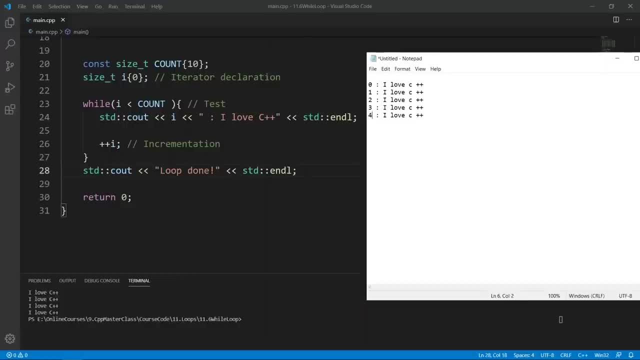 going to keep doing this and we're going to increment again. we're going to get a 5.. the test is going to run again. we're going to say: is 5 less than 10? that's going to be true, of course, and we're going to run the code to print: 5. i love c plus plus. we're going to increment again to get a. 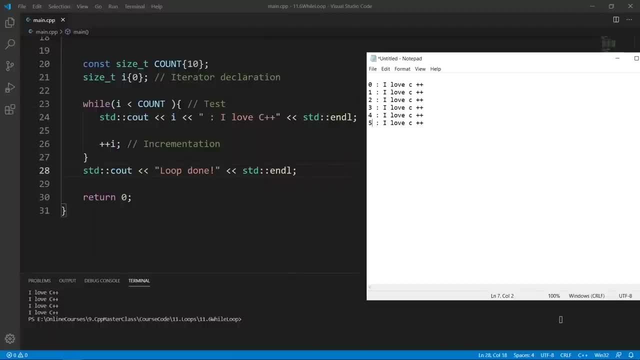 6.. we're going to run the test. we're going to say: is 6 less than 10? that's going to be true, of course again. and we're going to print sets. i love c plus, plus, and we're going to increment to get a 7.. 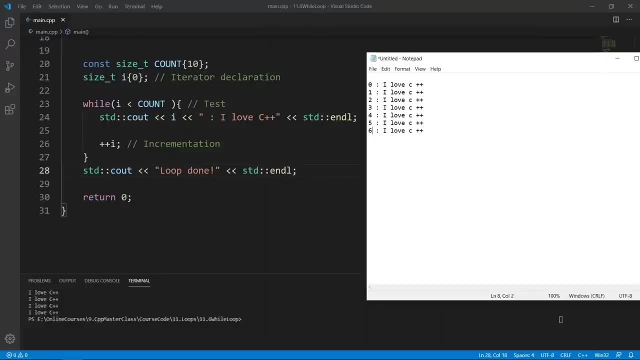 we're going to run the test, our iterator. we're going to say: is 7 less than count? that's going to be true. we're going to print the message again and say: 7, i love c plus plus, and we're going to increment again to get an 8. we're going to say: is 8 less than count? that's going. 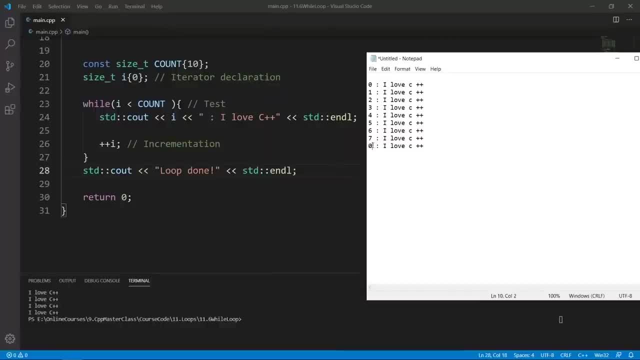 to be true. we're going to fall in the body and say: 8, i love c, plus plus. we're going to increment to get a 9.. we're going to run the test against our 9.. of course, 9 is less than 10, so that's. 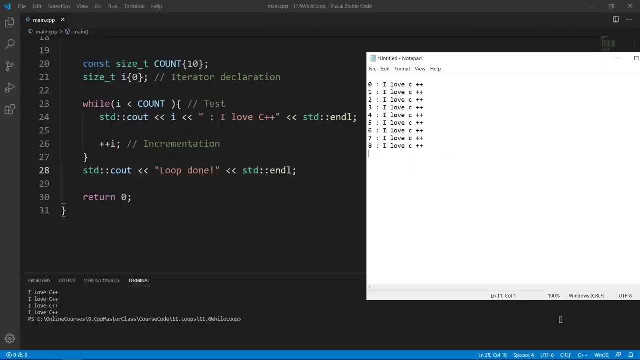 going to be true. we're going to fall inside and we're going to say: 9, i love c, plus, plus, and after that we're going to increment again and we're going to get a 10.. now, if we run the test, we're going to say: is 10 less than 10? and that's going to be false, because 10 is not less. 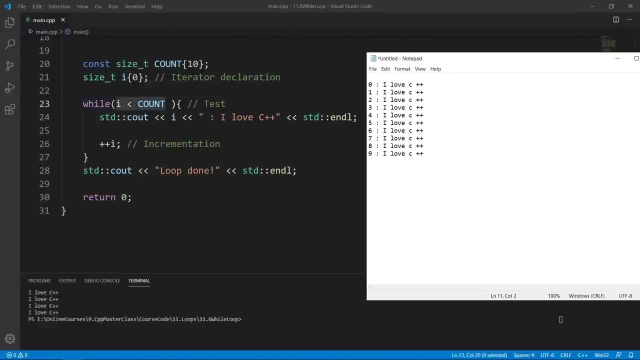 than 10. and if the test here fails, we're not going to fall in the body of the loop, control is going to fall at the end of the loop body and we're going to print loop done. that's what we're going to say here. we're going to say loop done and our loop will have run 10 times by the time. 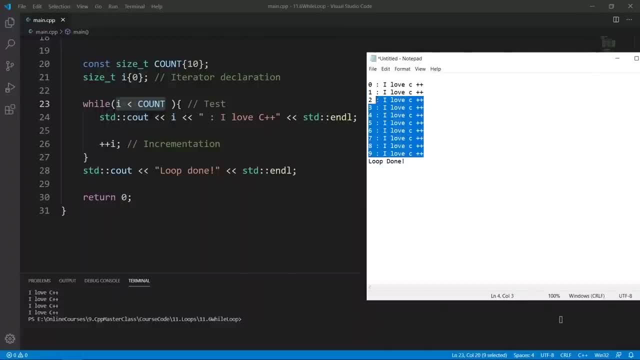 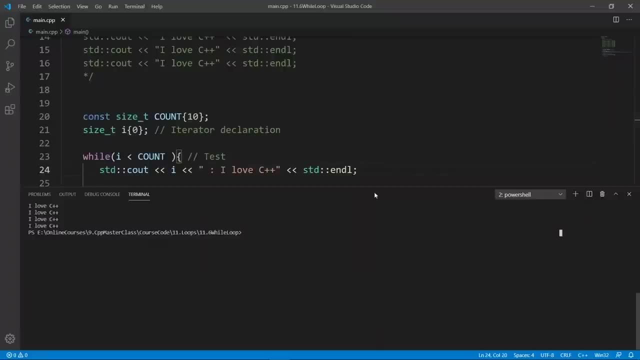 we print this loop done message here. if you count here, you see that the loop is going to run 10 times and it is going to say: i love c plus plus 10 times, which is really what we want. okay, i really had to show you this manually so that you can really see what is happening. but now we can build and run. 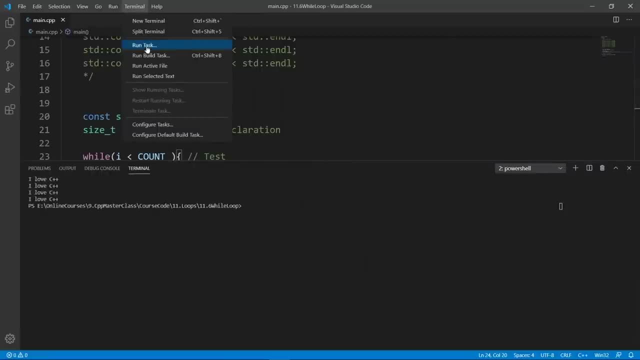 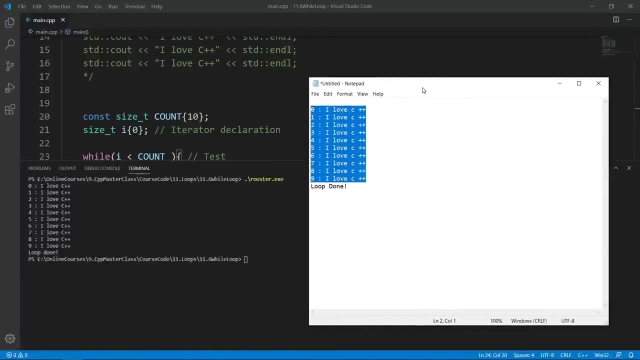 this and let the computer do the heavy duty of running this and showing us all these messages. so the world is going to be successful. of course, we're going to run rooster and it's going to exactly show the same thing we just came up in our trusty notepad file here. you see, it is the same. 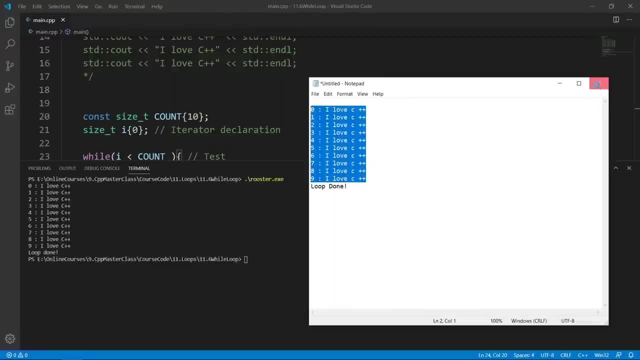 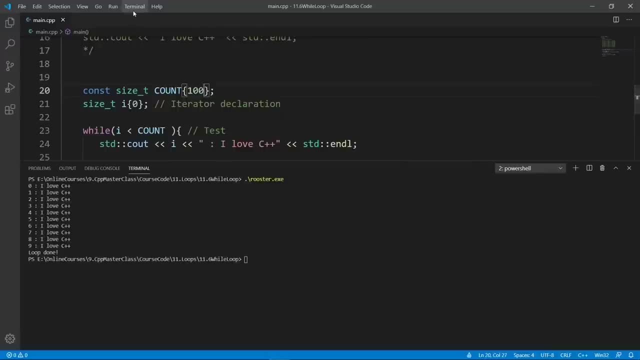 thing. but the beauty is that we don't have to do all these crazy computations again. what we can do is we can even change the count to 100, so it is going to run for 100 times, and that's pretty cool. so we can clear and run rooster and it's going to do that 100 times, and that's pretty fast. 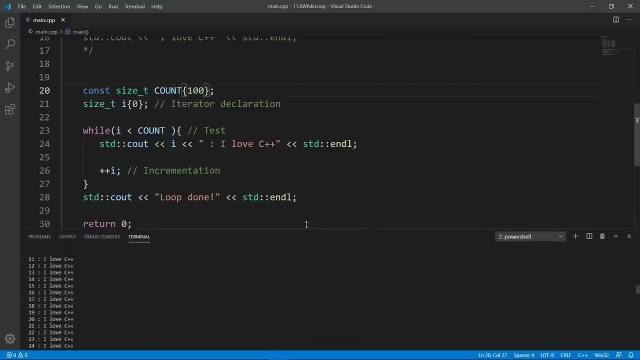 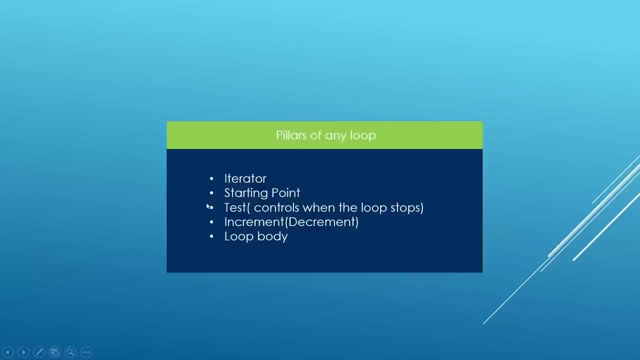 for computers. this is really all we had to share with you in this lecture. the main thing is to learn about the syntax of a while loop and again notice that we have these five parts that make up our loop. we have an iterator, we have the starting point, we have a test. 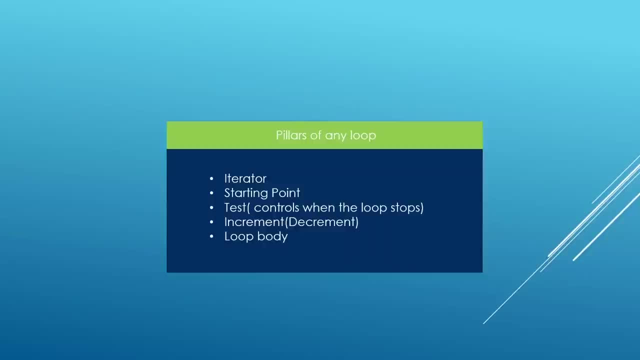 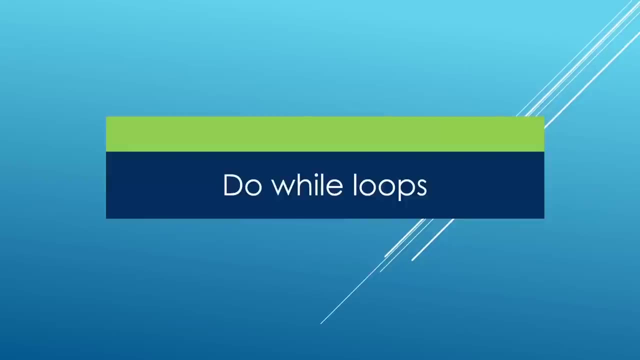 we have the implementation part and we have the loop body. it is just set up differently, with a while loop, like we can see. here in this lecture we're going to learn about do while loops, and this is yet another construct we have in c plus plus to do repetitive tasks. let's look at the syntax. here we have our 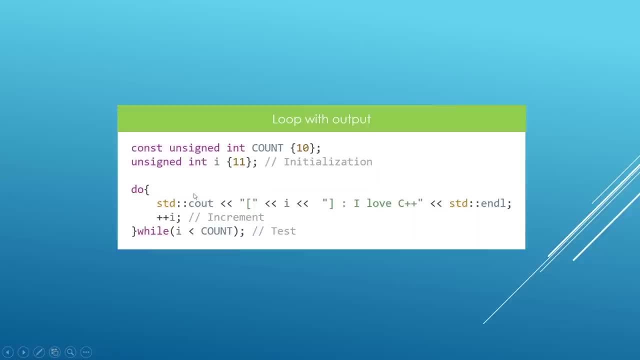 declaration of the iterator on the outside, and after that you're going to say: do you're going to put a pair of curly braces like this? you're going to put whatever code it is you want to run inside the loop, and then you're going to do your incrementation and after the closing, 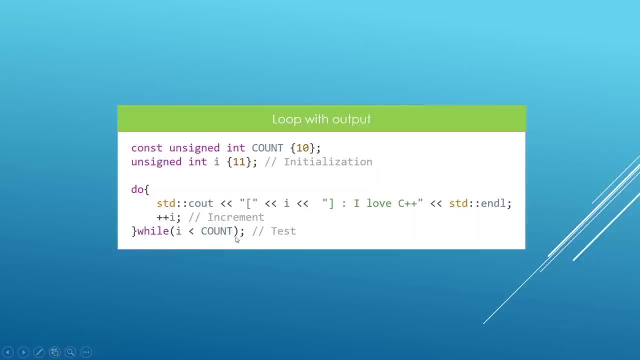 curly brace. you're going to say while and you're going to put in your test. this is really the structure. again, notice that we have those five parts in. this is the declaration of our iterator and we're going to initialize this in place, for example, if we want to do that. after that we're. 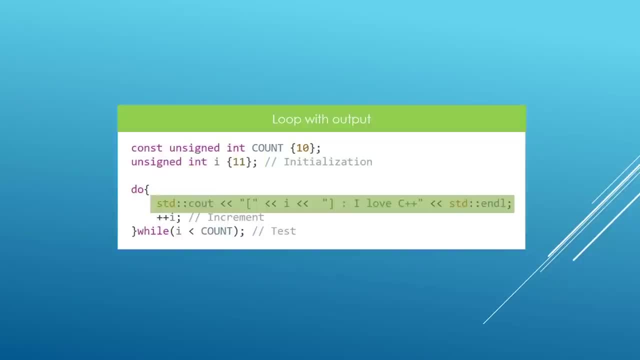 going to fall in the body of the loop and after that we're going to do the incrementation. after we run the code. it is we want to run in the body of the loop and then we're going to do the test, and the special thing about a do while loop is that it is going to run first. 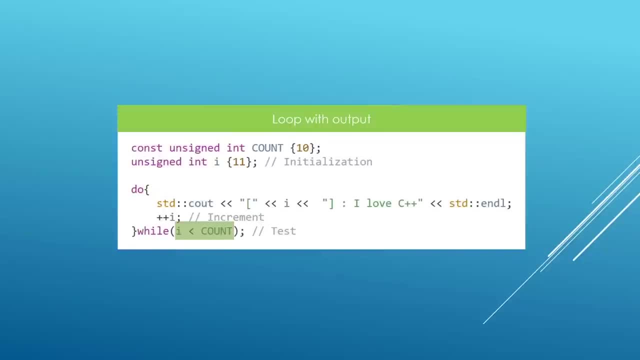 and then do the test. last- and this is really something you need to be careful about- make sure that when it runs, it is doing whatever it is you want to do, because the test is going to run after your code has actually run and you can tweak this to do whatever it is we want it to do. 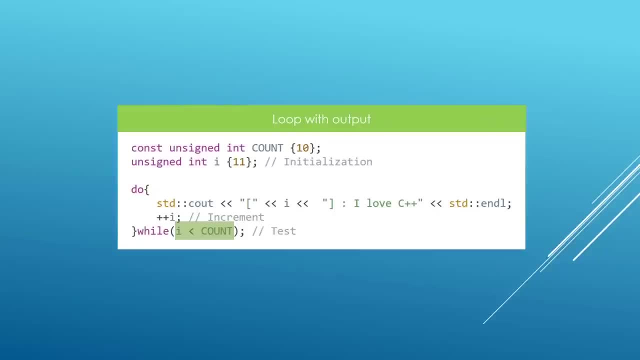 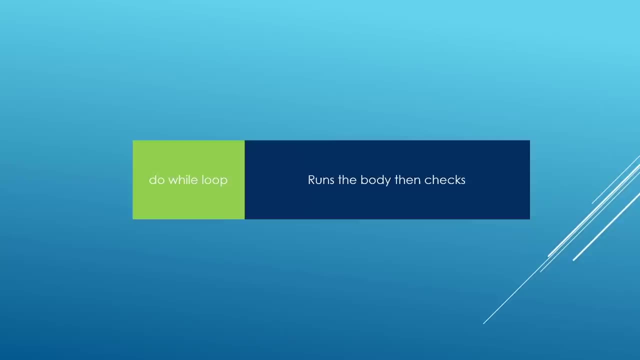 as we are going to see when we hit visual studio code in a minute. okay again, one thing you need to keep in mind is that the do while loop is going to run the body of the loop and then do the check or the test, and that may come in handy in some of the applications you'll be. 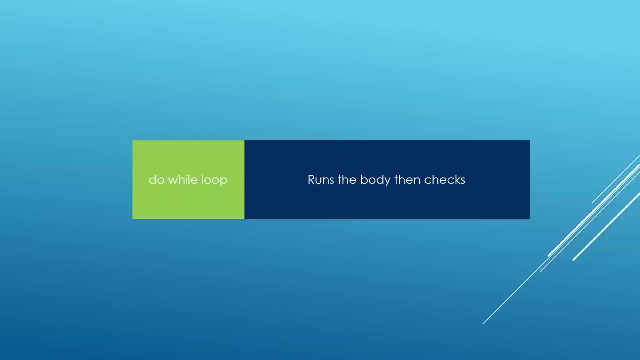 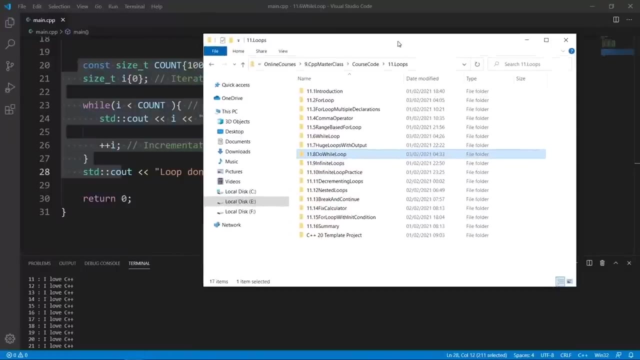 doing within your career as a c plus plus developer. okay, this is really the syntax we're going to be using. we're going to head over to visual studio code and play with us. okay, here we are in our working folder. the current project is going to be do, while loop we're going to grab. 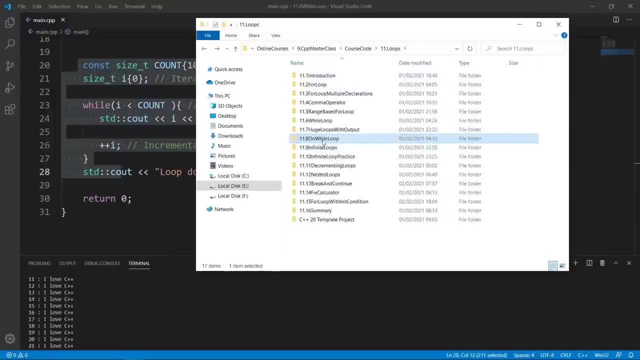 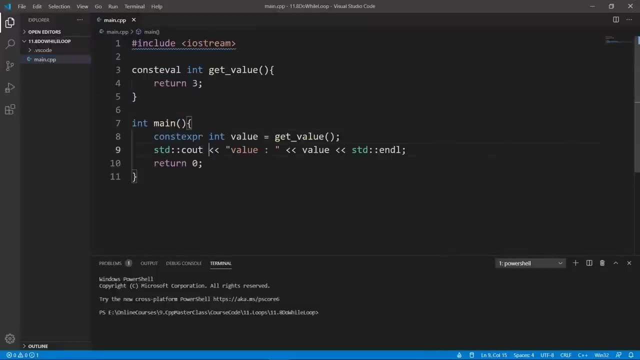 files pretty fast and we are going to put them in our current project. let's open this up and put them in there, and we are going to open this in visual studio code. do while loop is our project. we're going to open this and our main cpp is opened up, so let's remove whatever it is we. 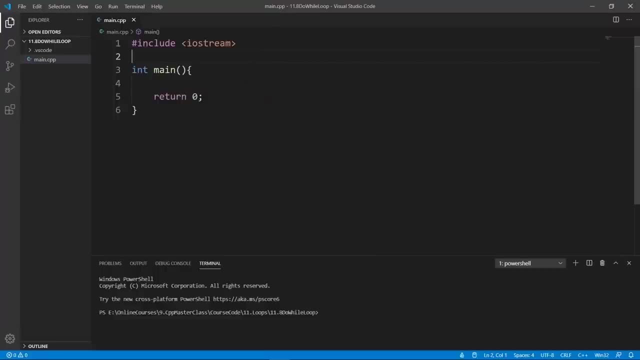 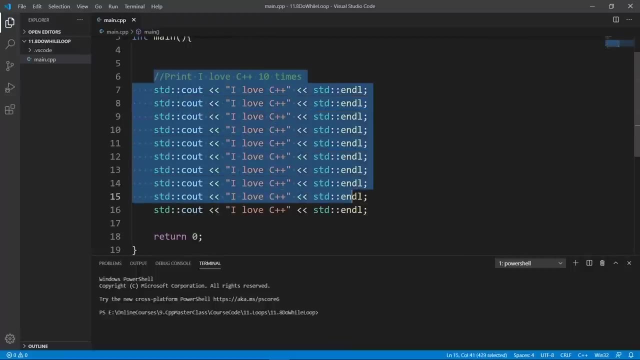 don't need, and we are going to show you the bad way to do things. the bad way to do things is typing your code to do things manually if you want them to be done multiple times, and this is something bad. if we work this and run, we're going to go down and run. 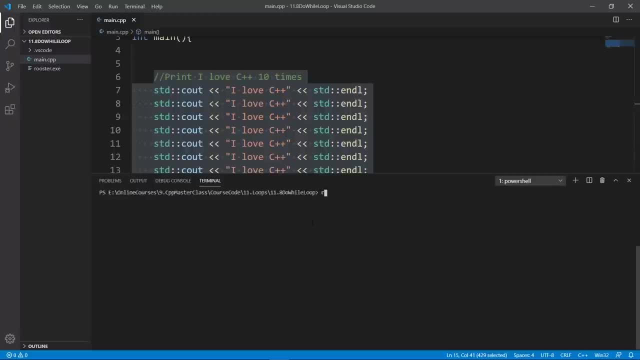 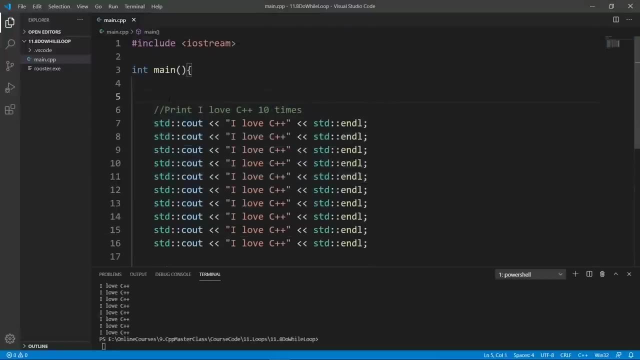 this clear. not, that's gbrush. we're going to run rooster and we're going to get i love c plus plus 10 times, and you don't want to do something like this. what we want in this lecture is to use do while loops to solve this problem. we're going to comment this out because it is really bad. 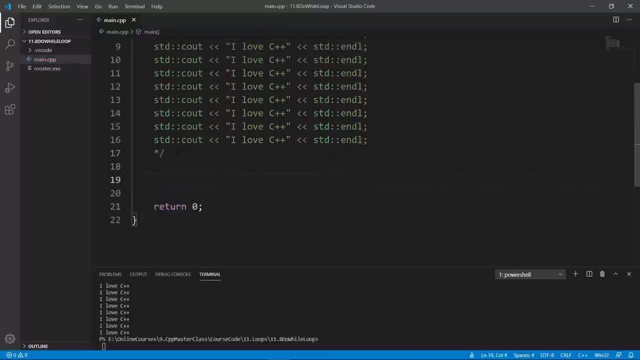 and we're going to go down and set up our do while loop. the first thing we need to do is to set up the count, because we want to store this in some variables. so we're going to say const and count and we're going to put in our value. let's put in a tan. 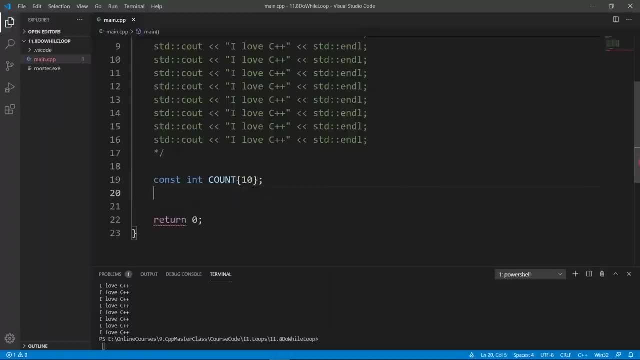 not 190, we're going to say 10 times and we're going to set up our iterator. we're going to say size t and we're going to say i and initialize this with our starting point. we're going to start from zero and what we're going to do is say do. 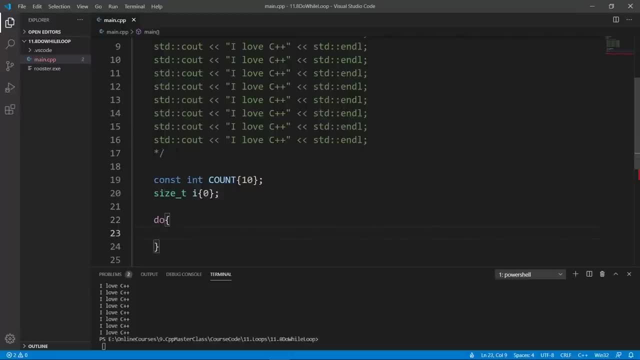 and put a pair of curly braces and inside this pair of curly braces we're going to put whatever it is we want to do multiple times. so we want to print: i love c plus plus. so that's what we're going to say, we're going to put in the current iteration and we're going to put a column and say: 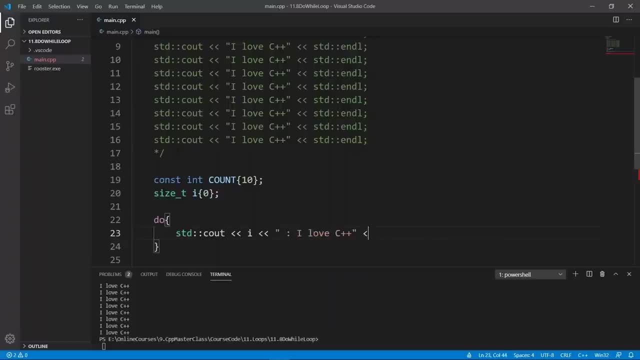 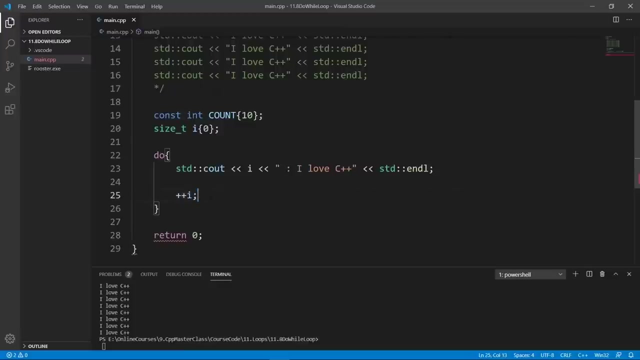 i love c plus plus, and then we're going to jump to the new line with s-t-d-e-n-d-l, and after that we are going to say i plus plus i, and this is going to be the part that moves our iterator to the next. 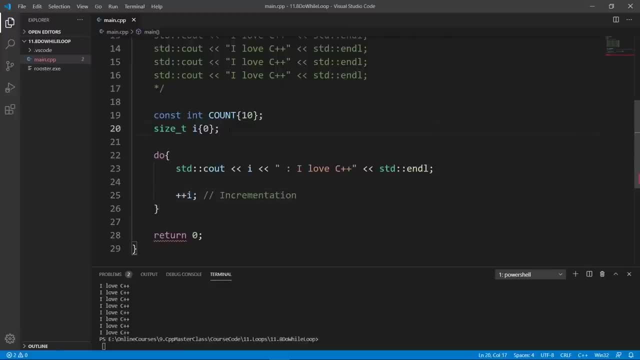 step. this is going to be the implementation and this is going to be the iterator declaration, and after the closing brace we need to say our test. so we're going to say while and we're going to put in our test here and we want to keep doing this as long as i is less than. 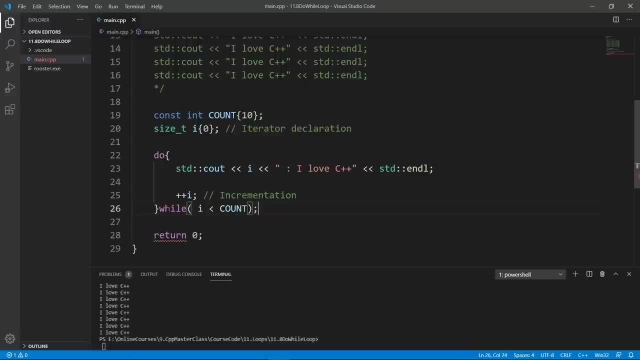 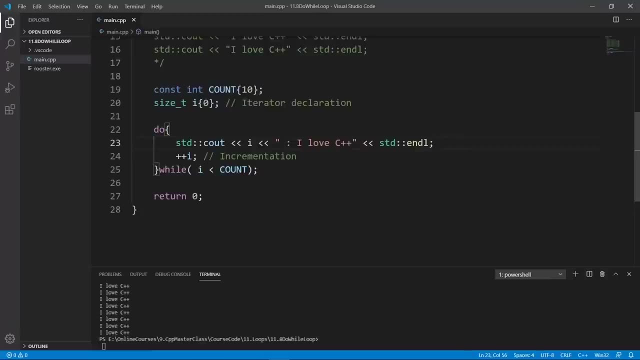 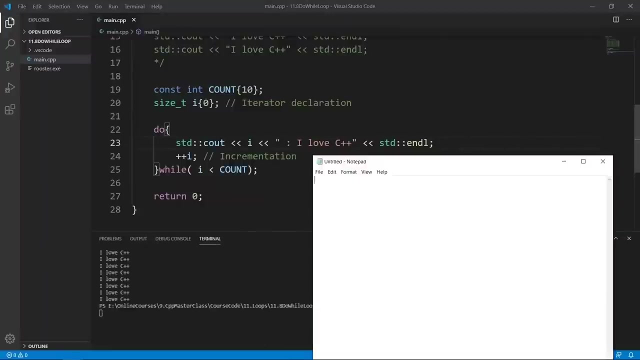 count, of course, and we're going to put in our closing semicolon here. now. this code is going to run 10 times, but let's go through how it's going to run so that you can really see everything that is happening here. okay, so when this code here is run, we're going to hit the. 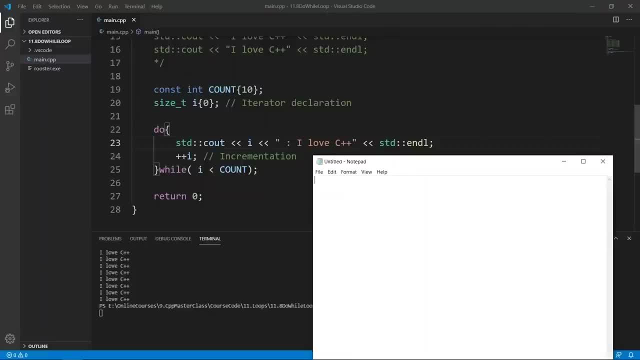 initialization line. here we're going to declare i and we're going to put in a zero, we're going to say do and inside we're going to print whatever we have in i and say: i will say: i love c plus plus. so we're going to say zero, because i is zero at this point, and we're going 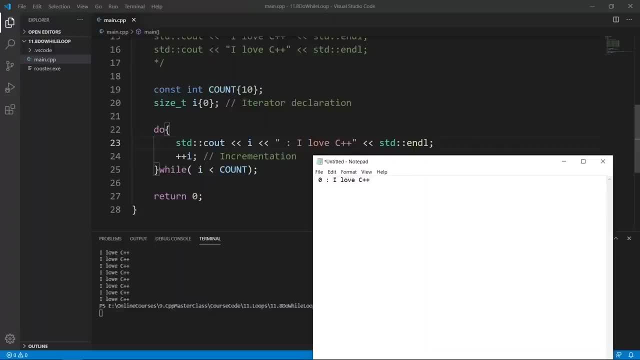 to say: i love c plus, plus, and after that we're going to increment, i is going to become one and we are going to do the test. at this time we're going to say: is one less than 10? that's going to be successful. so we're going to run the body again. 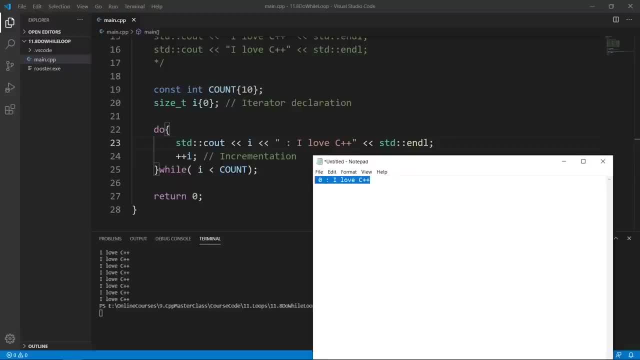 and we're going to say one: i love c plus plus. let's copy this and print this again so that we don't have to type this all the time. we're going to say one i love c plus plus, and after that we're going to run the incrementation part again, so we're going to get a two inside i we're. 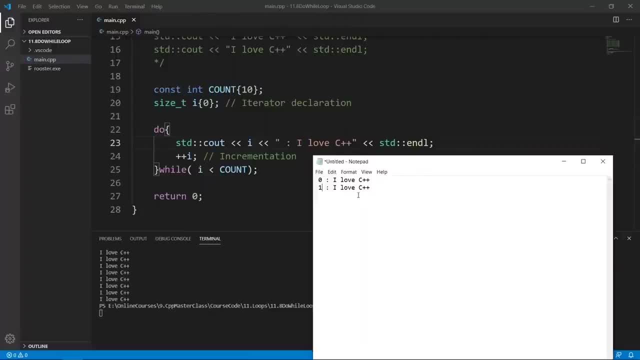 going to test and say: is two less than ten? that's going to be true. so we're going to run the body again and print two- i love c plus plus. and we're going to increment to get a three index. we're going to run the test against our three: is three less than ten? that's going to be true. so 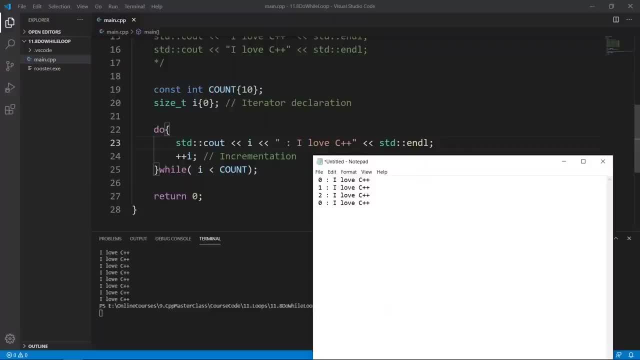 we're going to fall in the body again and print three. i love c plus plus. let's do that. we're going to do the incrementation. we're going to get a four inside this. i variable here. we're going to run the test. we're going to say is four less than ten? that's going to be true, of course, we're going. 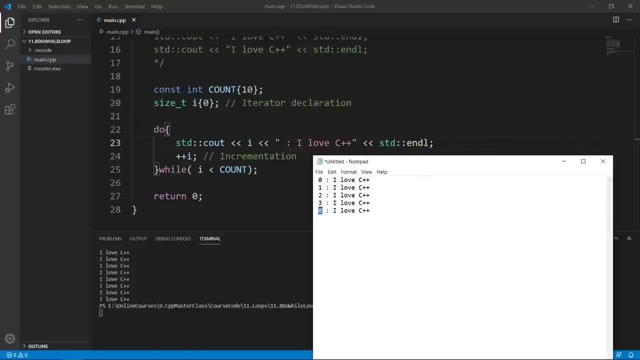 to say four, i love c plus plus when we fall in the body again. we're going to do the incrementation and get a five. we're going to do the test is five less than ten. that's going to be true. so we're going to fall in the body again and say five, i love c plus plus. 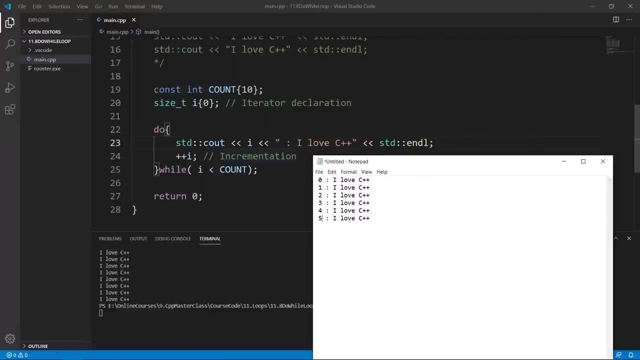 let's say that we're going to increment again. we're going to get a six. the test is going to run and we're going to say: is 6 less than 10? that's going to be true again. then the body is going to execute and say: six, i love c plus. we're 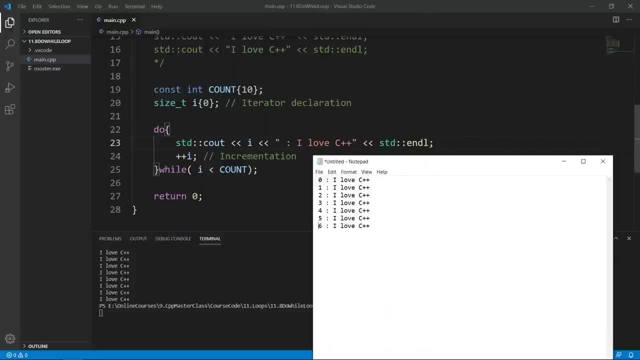 the incrementation and get a 7.. We're going to run the test against our 7.. So we're going to say: is 7 less than 10.? That's going to be true. We are going to fall in the body again and say, 7, I love. 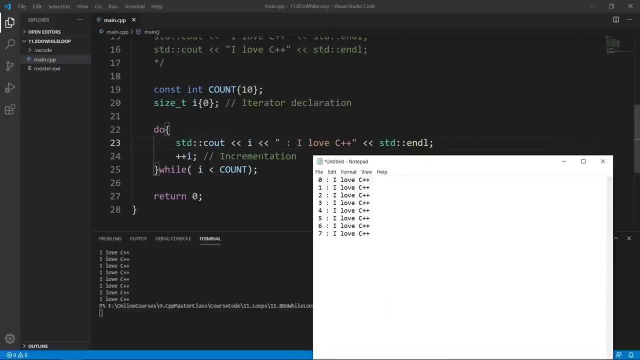 C++. We are going to do the incrementation. We are going to get 8.. We're going to say: is 8 less than 10.? That's going to be true. We are going to fall in the body again and say, 8, I love C++. 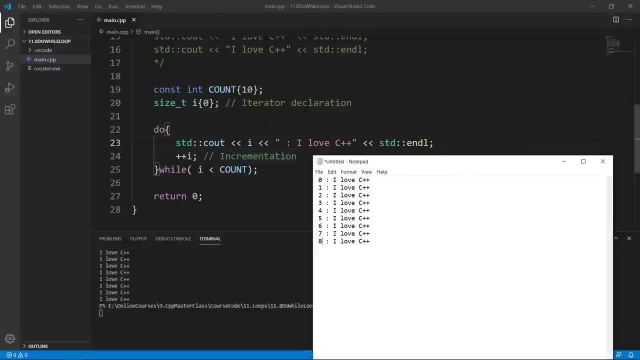 We're going to do the incrementation, We're going to get a 9 and we're going to run the test. We're going to say: is 9 less than 10.. That's going to be true. So we're going to go inside and say: 9, I love. 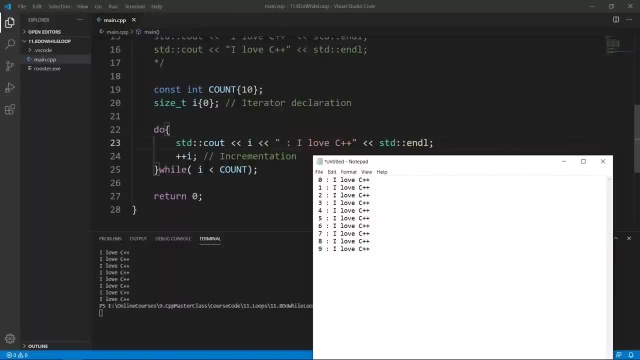 C++ and we're going to do the incrementation again. Now we're going to get a 10 and the test is going to say: is 10 less than 10, and that's going to be false. Now the test is going to fail. 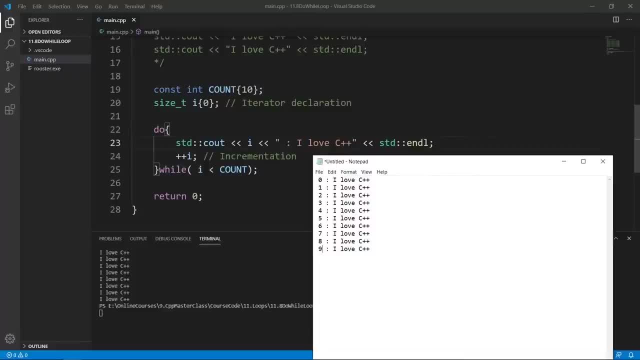 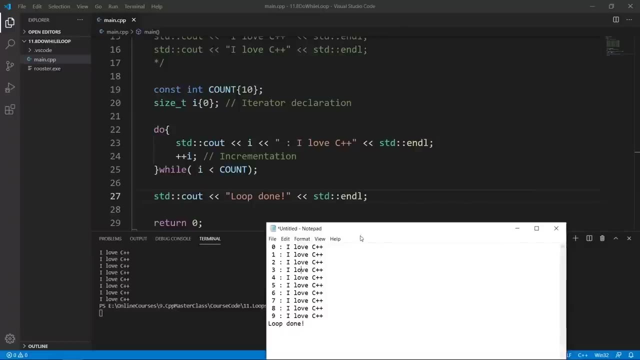 and we're going to fall after the while loop here. So if we had a statement here that said stdc out, loop done, we would print that, We would go down here and say loop done. and this is what we're going to get if we run this program. and again, I encourage: 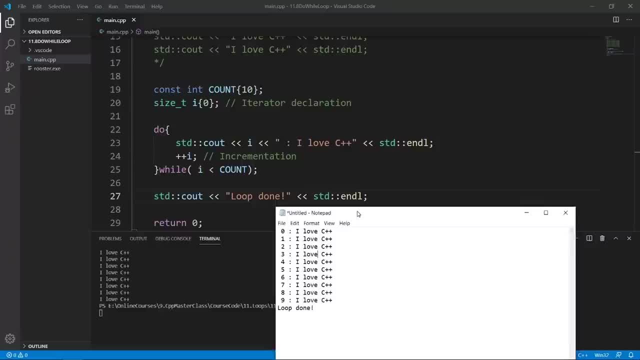 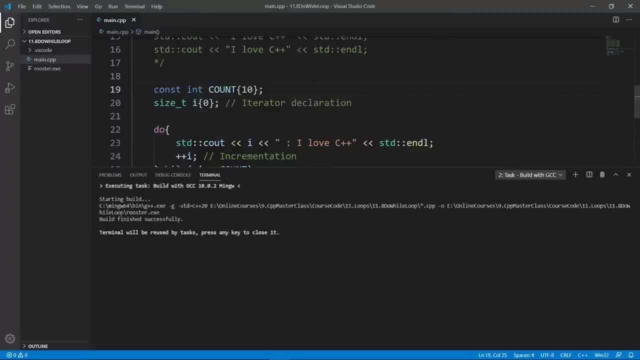 Do the heavy work for us and run this dense multiple times. the build is going to be good. so what we're going to do, we're going to say: clear and run rooster. and it's going to say exactly what we expect. i love c++ 10 times and then it's going. 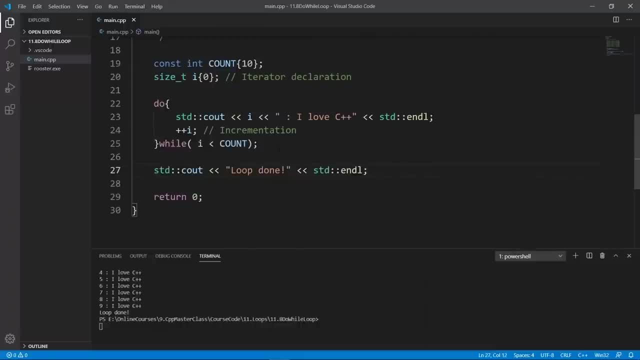 to say: loop done, Okay. one thing I want you to see is that the Do-While loop runs before it does the test, and this may cause crazy things happening in your program if you're really not careful. let's say that you wanted this program not to run and initialize this thing with a zero for. 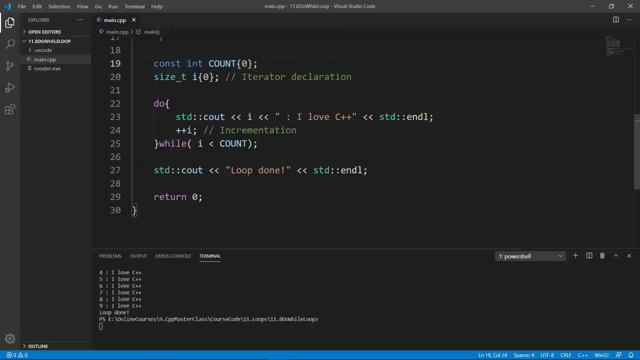 the count. so it's going to run zero times. but that's not going to do what you expect with a do while loop, because it runs things before it does the test. so if you run this program it's not going to just say loop done, it's going to say i love c++ and have zero value in here. 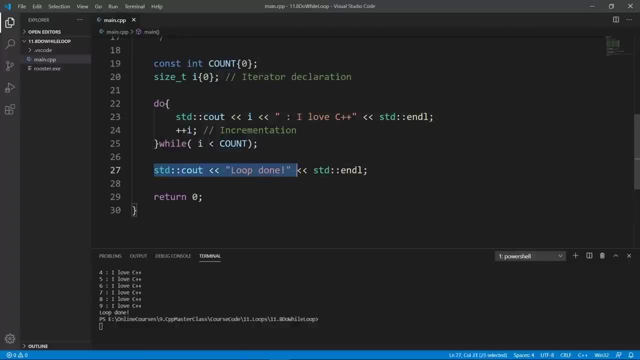 and it's going to say loop done. but that's not going to be probably what you intended by putting a zero in here. you put a zero in here if you want this code to run zero times or the code in the body not to run. that's another way to say that, but in this case, a do while loop is not. 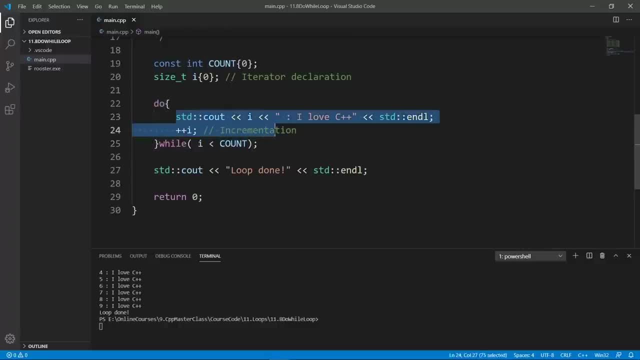 going to do what you expect, because it runs before it does the test here. let's build this and show you this. so we're going to go Succesful and we are going to clear and run rooster. you're going to see that it's saying. 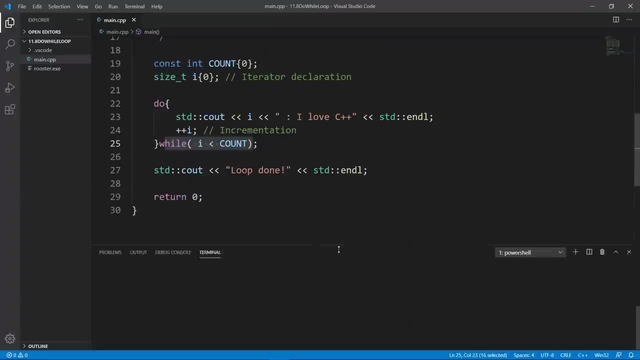 zero. i love c++ loop done. it is running even if we set our count to zero here. so be sure the do while loop is doing what you want. but if you are careful about this you're going to have no problems. and if you want the loop to actually not do anything when you have zero count, in here you. 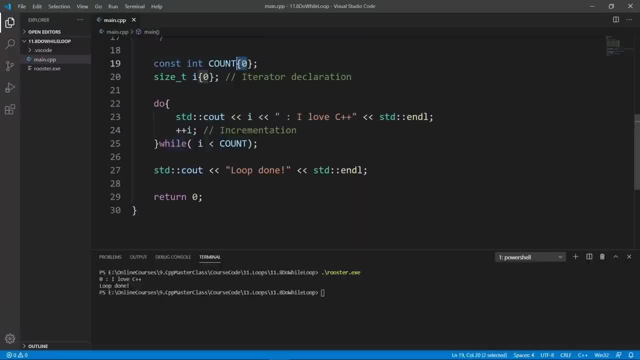 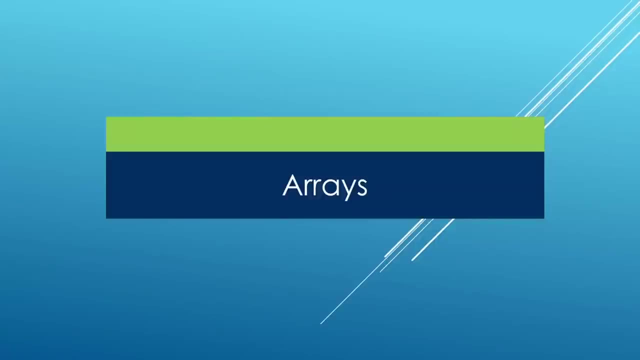 can use the while loop to run it and it will run the test, and it will run the test and it will run the loop or the full loop, like we have seen before. i would like to welcome you in this new chapter, where we're going to be learning about arrays, and arrays are a way to set up collections. 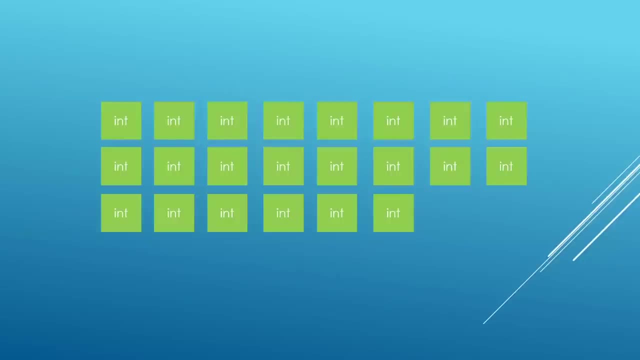 in our c plus plus program. so far we have been working with single variables. for example, you have a bunch of integer variables. you can even have 10 or 20 variables of integer type and that's going to be fine. but sometimes you don't want to manage all these variables and you don't want to. 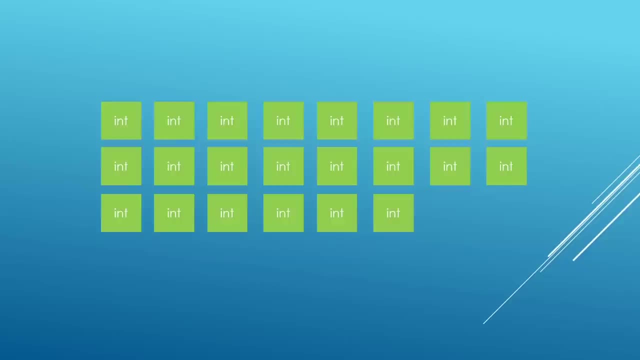 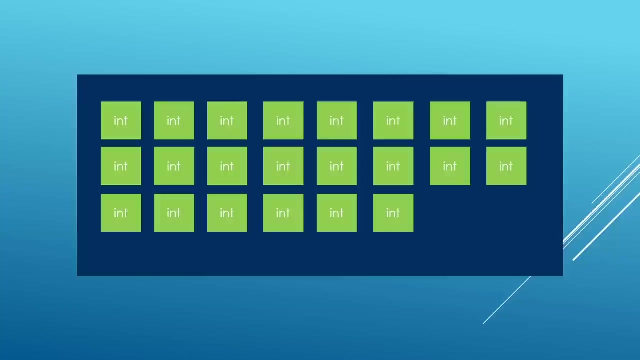 manage all these variables. it is really desirable to group all these variables into one single unity and manage them as one single entity, and we can do something like this: group them together and give them a name so that we can refer to them or manipulate them under this name here and c plus. 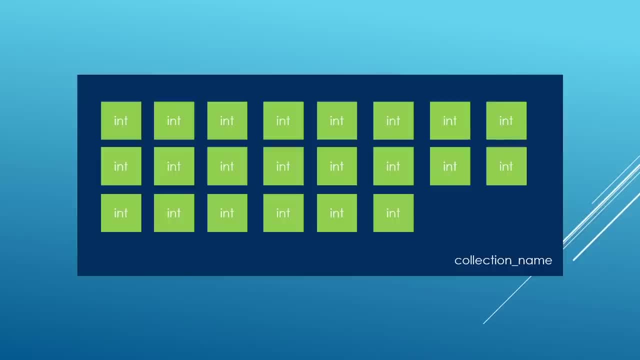 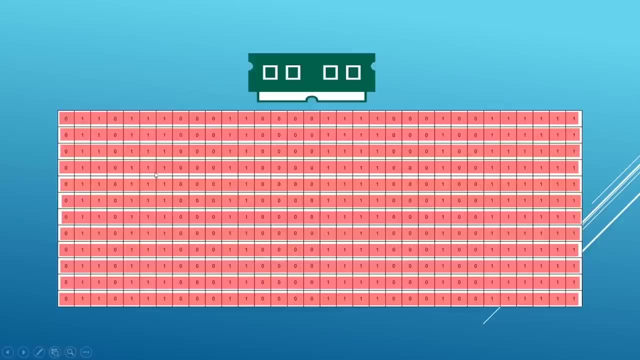 plus has the array construct to help us do this. because so again, if you look in memory how things are laid out, you're going to have a bunch of variables and you're going to have a bunch of zeros and ones. for example, here, each red thing is a net. it is four bytes in size and it can be. 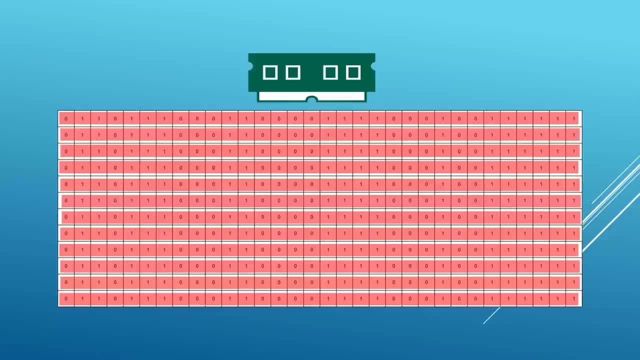 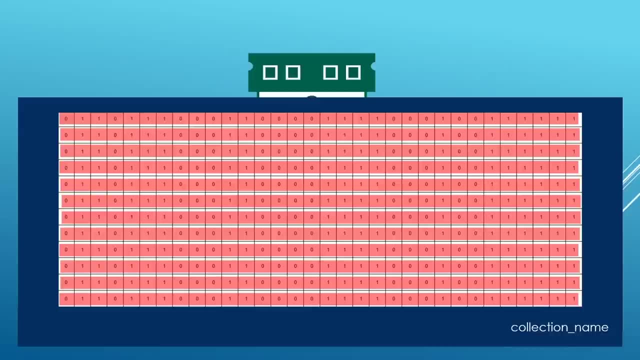 used to represent a net. so if we have a bunch of events like this, we might want to group them together and give them a name and manipulate them under this name. this is another way to look at what we just talked about. here and again, arrays are a way to do these kinds of things in. 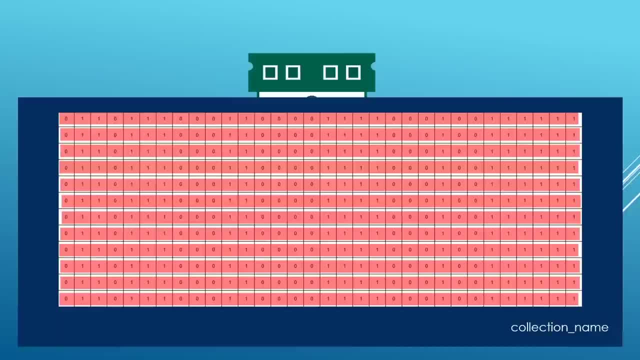 c plus plus, and we're going to be learning all about it in this chapter. we are going to be learning all about it in this chapter. we are going to be learning all about it in this chapter. we are going to stop here in this lecture and we are going to start and look at how you can declare and: 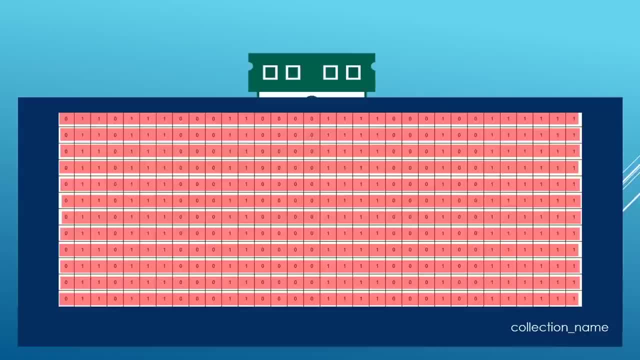 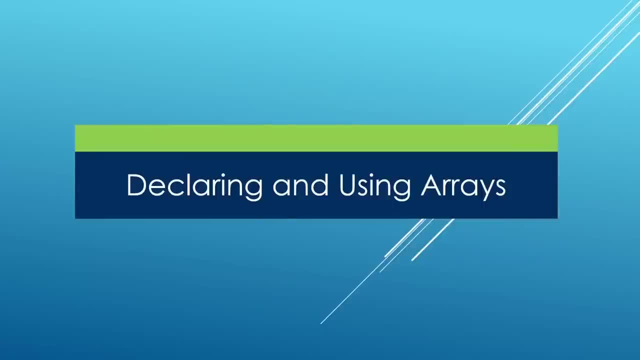 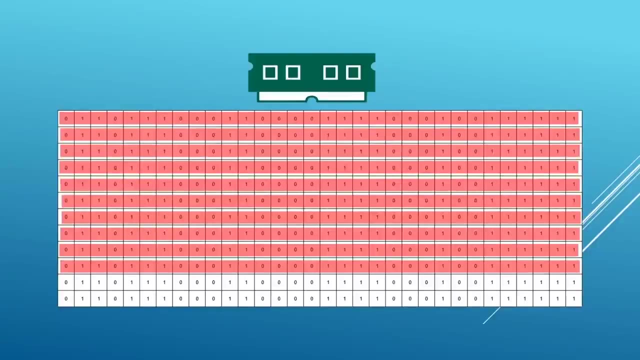 initialize an array. in the next lecture, go ahead and finish up here and meet me there. in this lecture we're going to see how we can declare and use arrays in our c plus plus program and again, arrays are a facility we have in the c plus plus programming language. 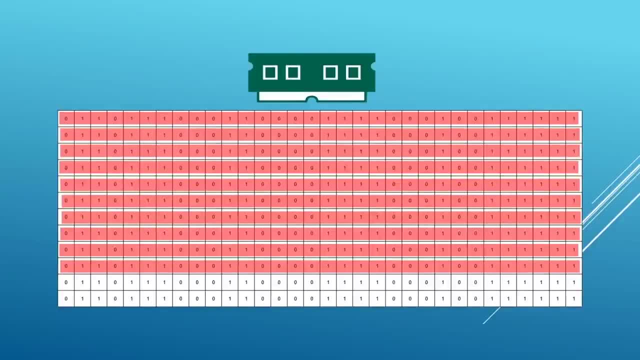 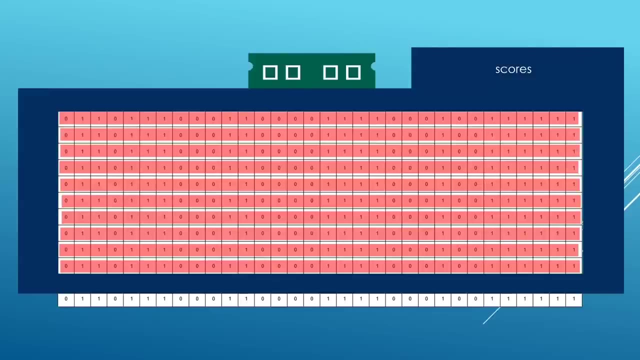 to group many variables together and manipulate them as a single unit. for example, here we have a bunch of integers in memory. each of these red things is going to be four bytes in size, so we can think of it as an integer and we can group them together and give them a name. we call them. 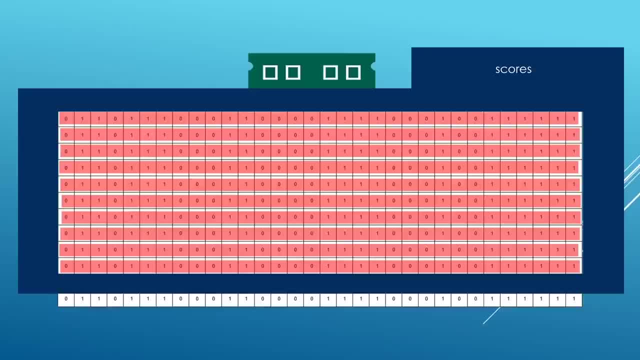 scores here and they are going to be living under that scores entity. so if we want to refer to each of these things, c plus plus provides an indexing system. so we can use angle brackets like this and refer to the first of these integers as zero. so we can go from zero all the way to nine here, but your array can even be bigger. 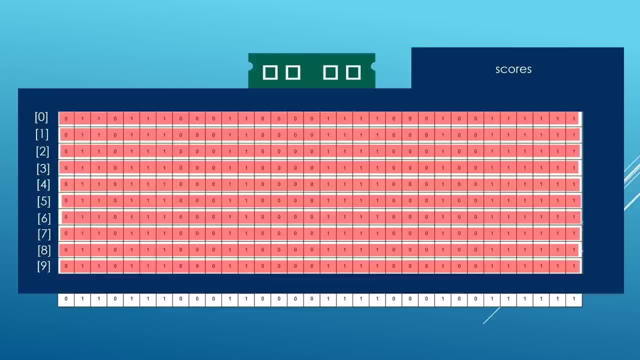 than this, many times bigger than this, and we're going to see examples of how we can do that. but this is an example of how you can take many variables, group them under one entity, give them a name and be able to reference each of these events that are under that entity. and now that 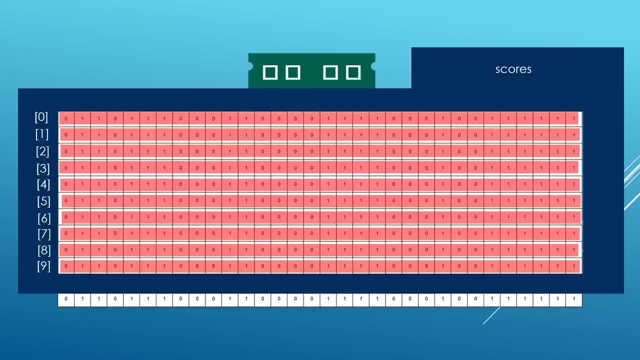 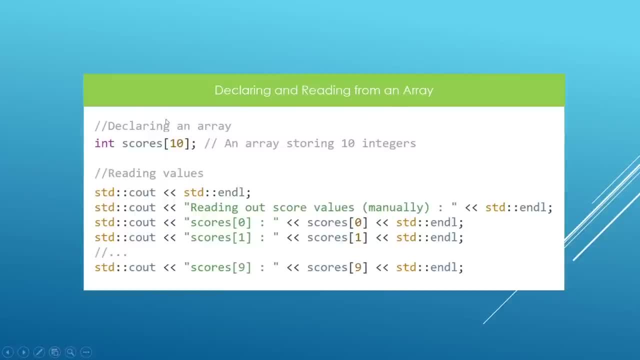 the idea is pretty clear. let's see how we can do this in c plus plus. the way to do. that is to say, and you have to specify the type of your collection, you have to specify the name after that, and then you're going to put a pair of angle brackets, like 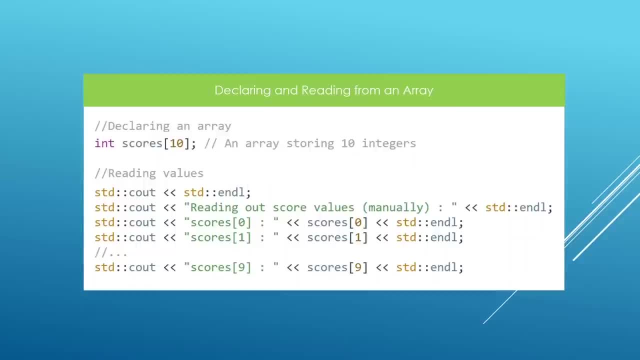 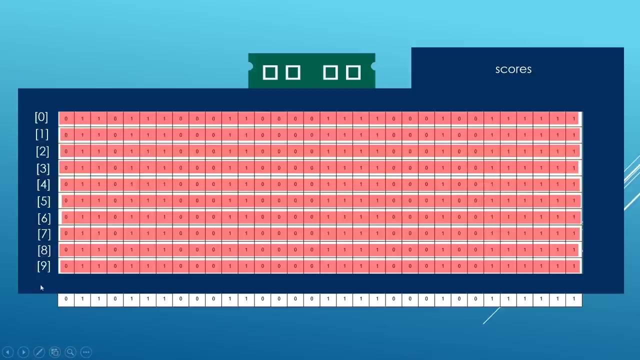 this and inside those angle brackets you can specify the size you want that collection to have or that array to have, and after this statement is run, we are basically going to have something like this in memory: we're going to have 10 integers, so if you count here, zero all the way. 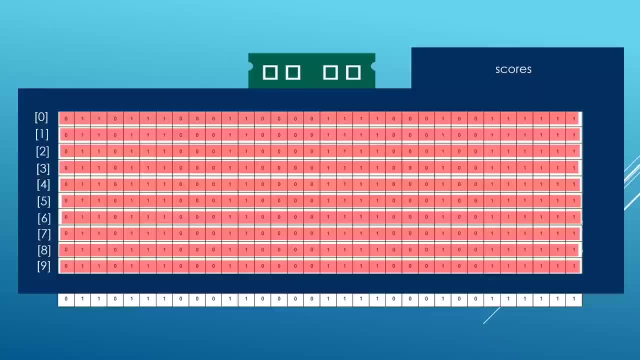 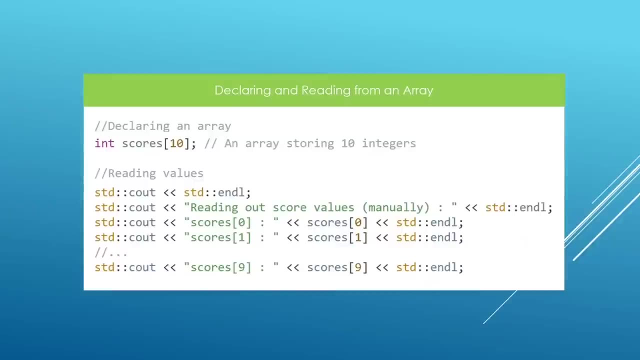 through nine, that's 10 integers. they're going to be grouped together under one logic entity. that logic entity is going to be called scores and we can go through that name to manipulate all these things that are in this entity. okay, after your array is declared and you have space for it, 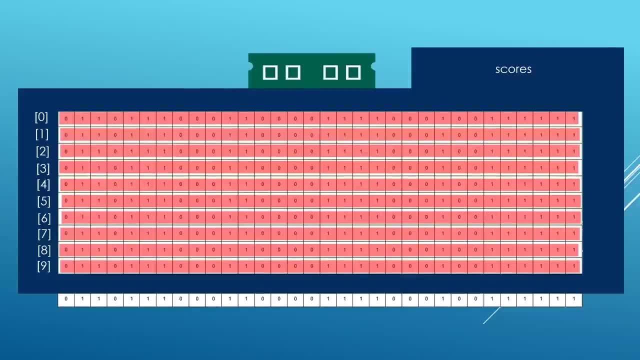 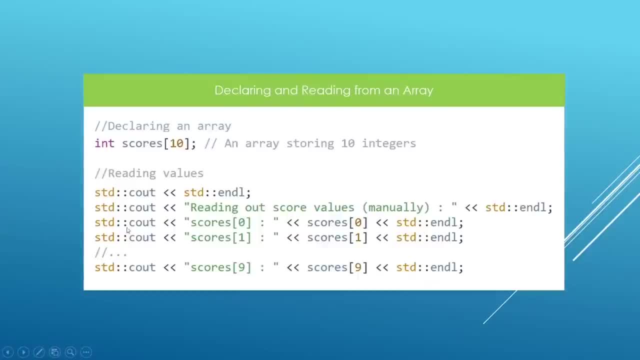 in memory, basically something like this: we need a way to read data from it and we're going to see how we can do that and it is what we have here. for example, if we want to print the first of these elements, we're going to say scores, angle brackets- and specify the index of the first element in that array or that collection of. 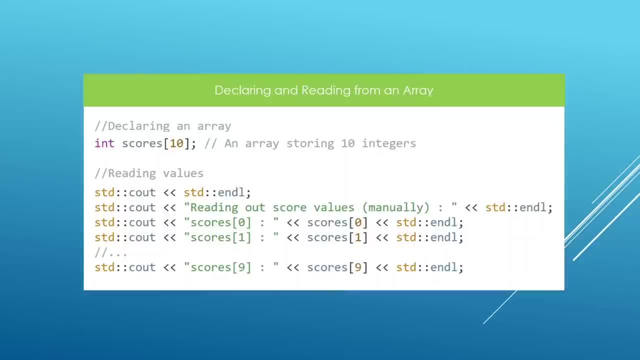 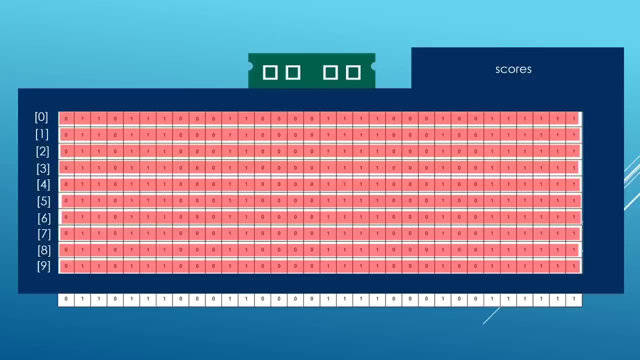 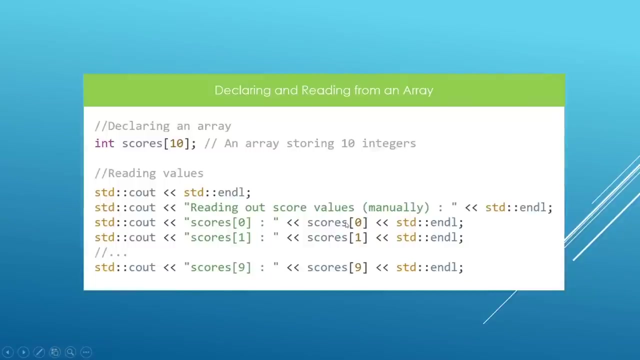 integers, that is called scores. okay, one thing you should really keep in mind is that arrays are indexed from zero. they don't start from one. so the first element is going to live at index zero. it's not going to live at index one. so here, scores zero is going to print the first element. 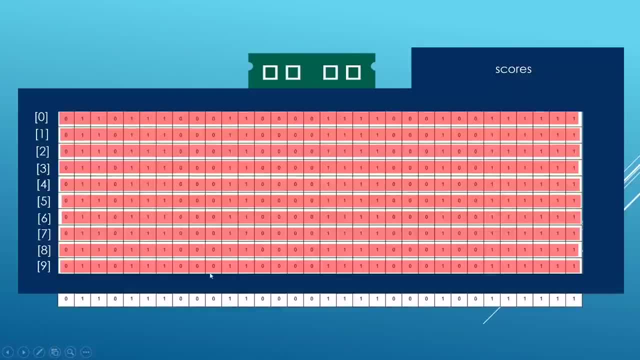 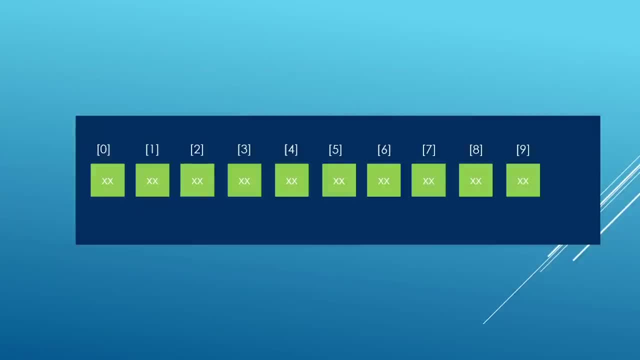 and scores nine is going to print the last element, which happens to be the last in our collection here of integers. okay, once our array is declared, it's not going to have data in it. there is going to be data in, but it's not going to be data that we put in. so we can think of this. 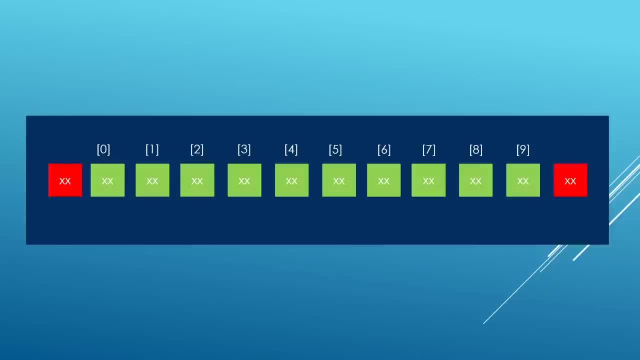 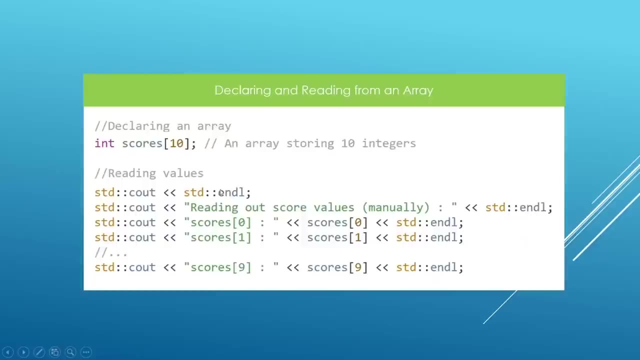 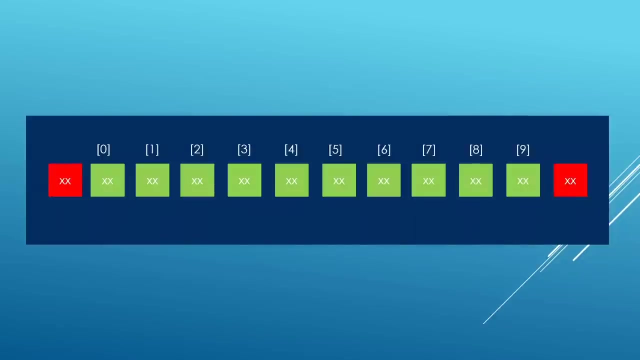 data basically as garbage. another thing i wanted to bring to your attention is that your array has clear boundaries. when we declare an array like this, notice that we specify 10 as the size of our array. it's only going to have 10 elements inside and you can see that we have, from index zero, all the 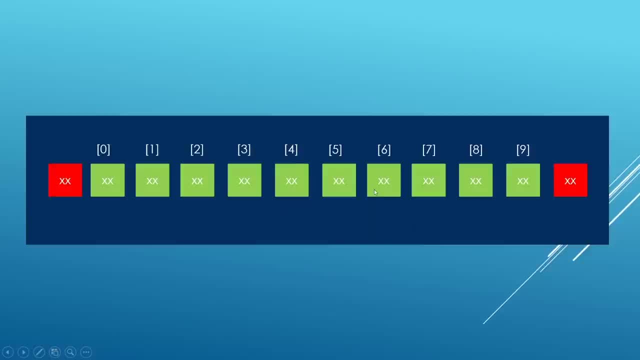 way to nine and inside we have garbage data. but we're going to fix that in a minute. what i want you to see here is that you can't try and read outside the bounds of your array c plus plus is funny in that it allows you to do that, but if you do that, you're going to get weird problems for. 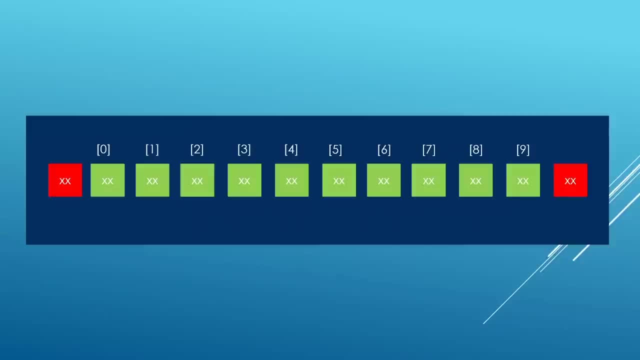 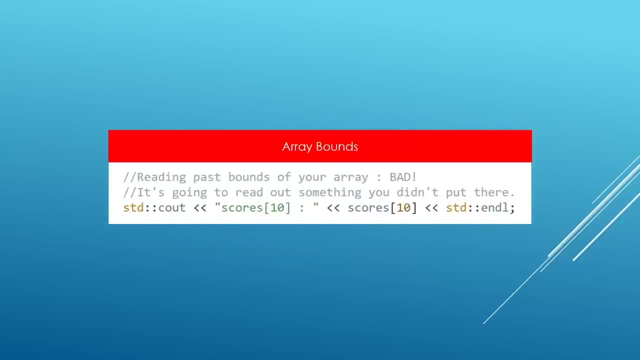 example, your program would crash or do something really bad. so you shouldn't really do this. be aware of the boundaries of your array and you can see that you can't read outside the bounds of your the boundaries of your array. if you try to read the data from the outside of your bounds, you may. 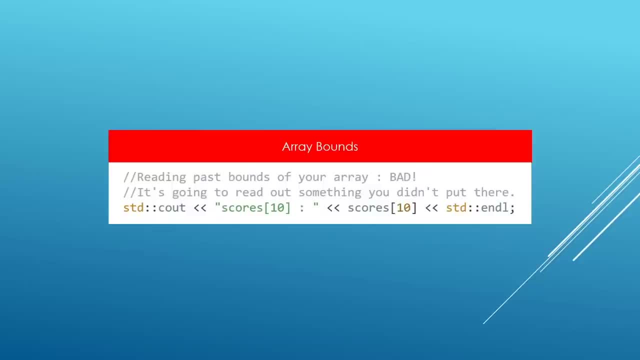 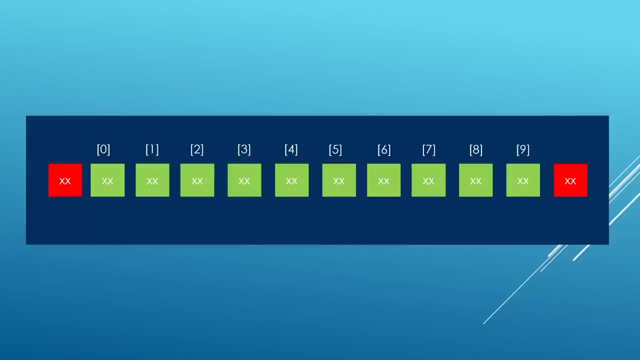 read garbage data. you may even cause failure of the operating system because you don't really know whose memory you're reading. it's not going to be memory that is allocated to your program. so array boundaries are something you need to keep in mind when working with arrays. okay, we just saw. 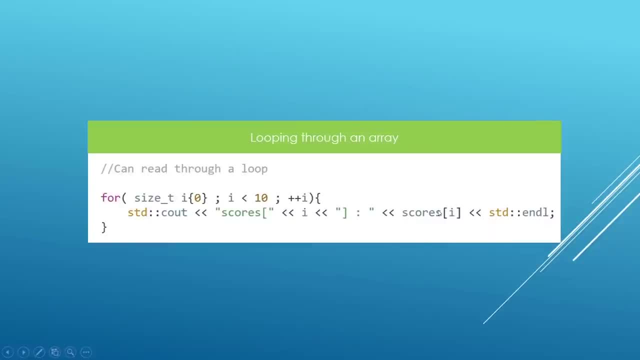 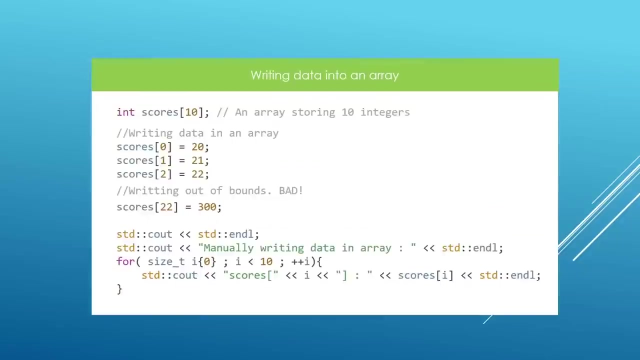 that we could read data from the array using this angle bracket syntax. we can even do that through loops and read all the elements in the array, and this is how we could do that, and you can see that the loops we learned about in the last chapter are starting to come in handy. okay, we have seen how we. 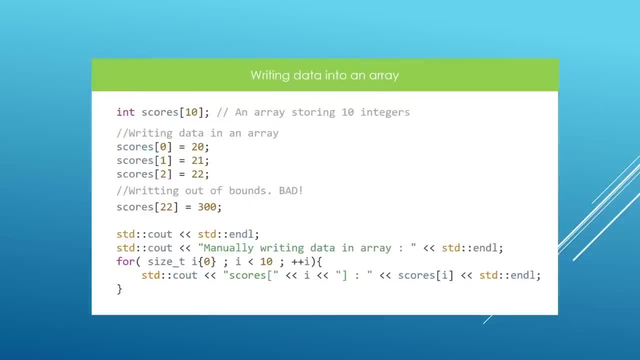 can read data from the array, but what if we want to put something back in? what if we want to write our own data in an array? well, the syntax is pretty much what you would expect. we also use this angle bracket syntax, but we're going to assign data to that. 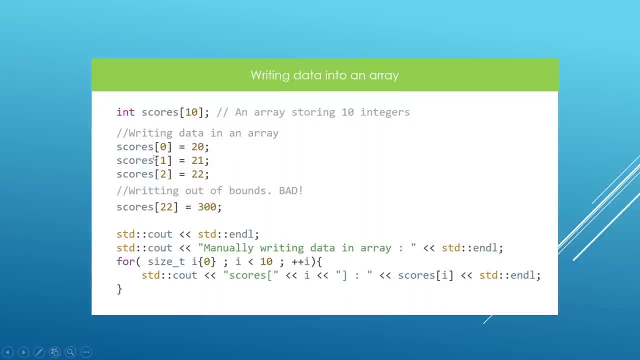 element in the array. for example, if we want to assign data to the first element in our array, we're going to say scores, angle brackets 0 and we're going to assign a 20 in it. and we can assign a 21 into the element at index 1 and a 22 in the element at index 2, and if we do that we're going. 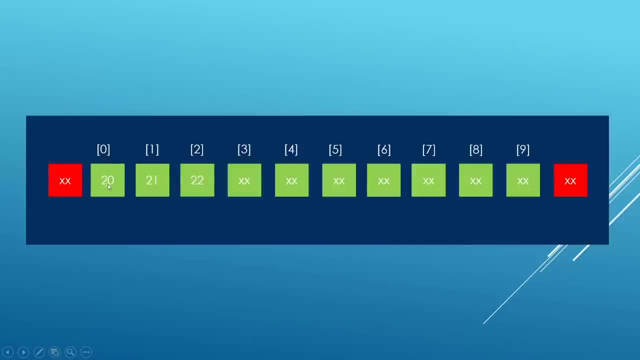 to have something like this in our array. so index 0, we have a 20, index 1, we have a 21, index 2, we have a 22 and the rest is still garbage because we didn't put in our data. we can also write data. 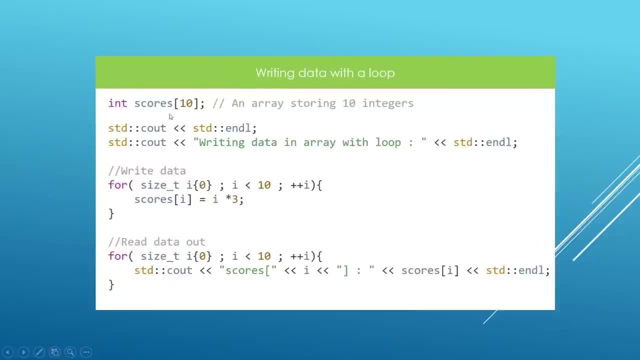 in a loop, for example. here we have our array declared and we're going to loop around putting data at different indexes. notice that the index is going to be the current iteration we are at. so this is a common way to do things in c plus plus and you need to be familiar with us and 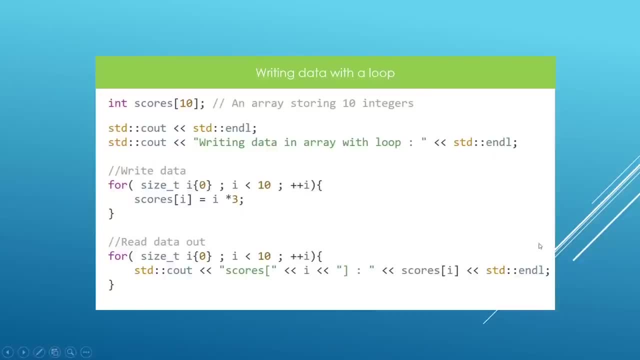 after we put in the data, we can read that back and make sure that it is the actual data that we put in. and we're going to have a chance to play with this in visual studio code in a minute, so don't worry if some of these things don't make sense yet. but again, the main. 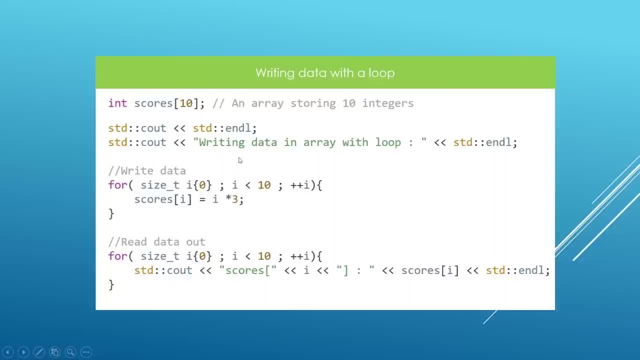 thing here is this angle bracket syntax. we can use that to either write data in the element of the array or read data from the element of the array, and this is the syntax here. scores angle brackets. i okay, so far our array has been declared and we didn't really put in data and there were. 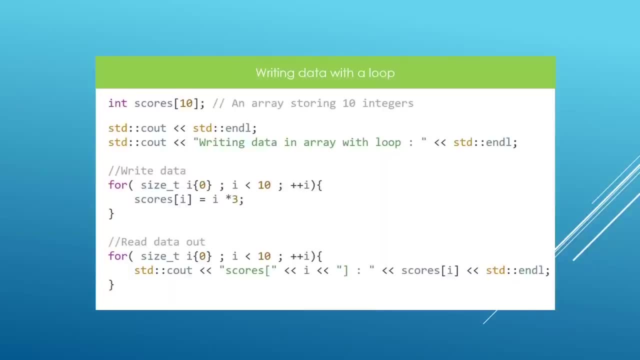 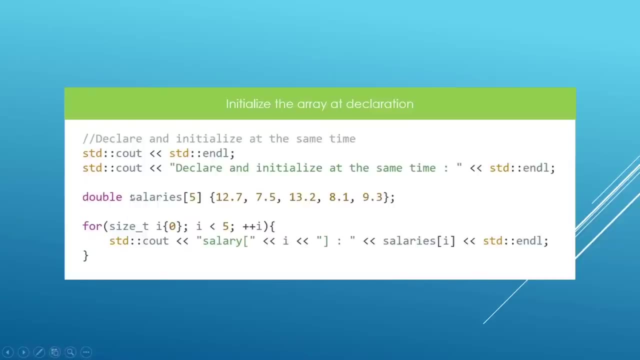 junk data inside. but there's a way you can declare an array and put data in in one single statement and this is how you would do it. here we have another array. it's going to be grouping double variables. we call the array salaries and we specify that it's going to be. 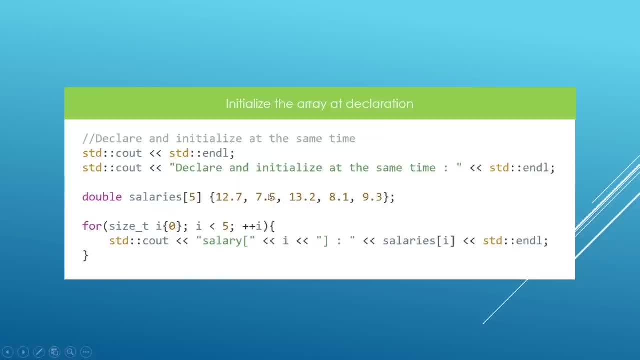 of size 5 and we can put these elements in a comma separated list using braced initialization like this, and it is going to work if we try to print it out. we're going to see these elements here and you see that we can read this using the same syntax we've learned about. 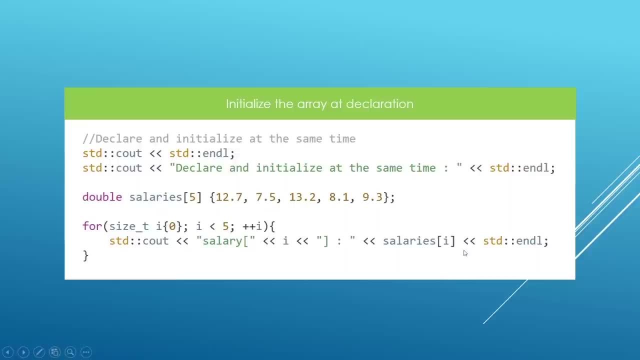 salaries. we say the array name, we do angle brackets and inside we put the index of the element we are reading from. and this index is coming from our loop here and it is going to work. you're going to get these elements printed out. this is pretty cool when initializing your. 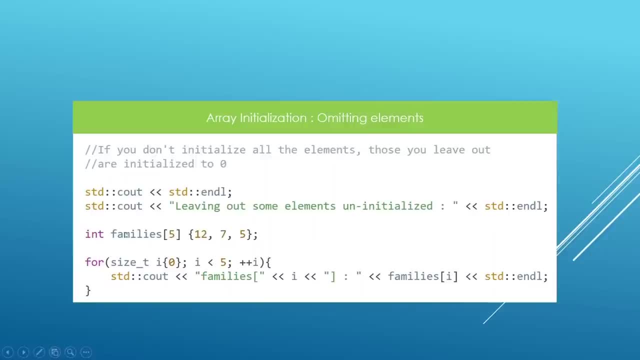 array, you can leave out elements. for example, here we have an int array. it is called families. it's going to be of size 꼰 five, but we are just putting in three elements. the rest are going to be initialized to zero. when we do things like this- and this is something you need to be aware of and we are going to try- 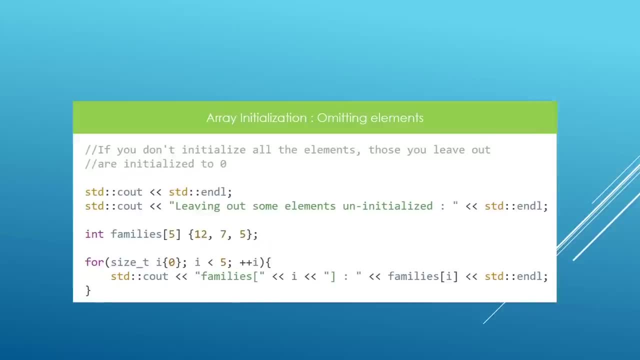 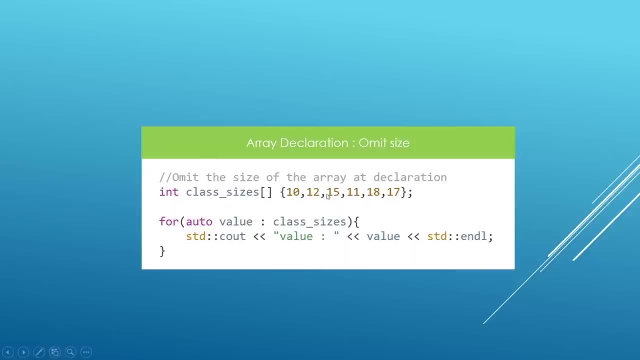 this out in visual studio code and you're going to see that this is actually true. it is possible to also omit the size when you are declaring your array, and the compiler is going to deduce the size from the elements that you initialize your array with. for example, here we have in one 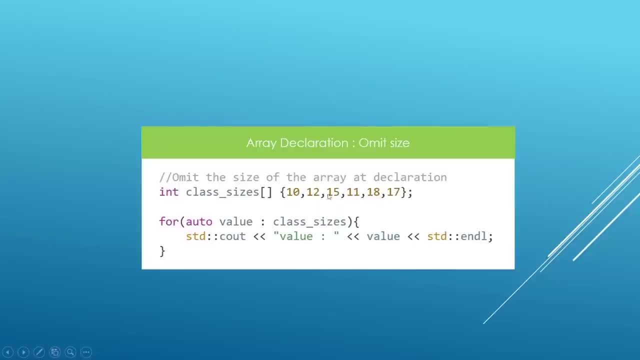 two, three, four, five, six elements. this array is going to have a size of six and if we print elements, we're going to get those printed out. notice here that we are using a ranged base for loop and, uh, hopefully you can see that it is easier to read data from a collection like this. 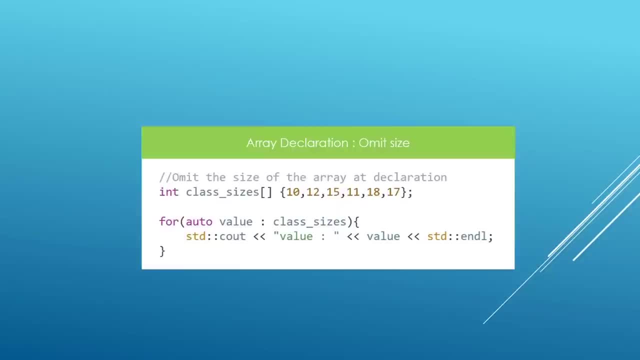 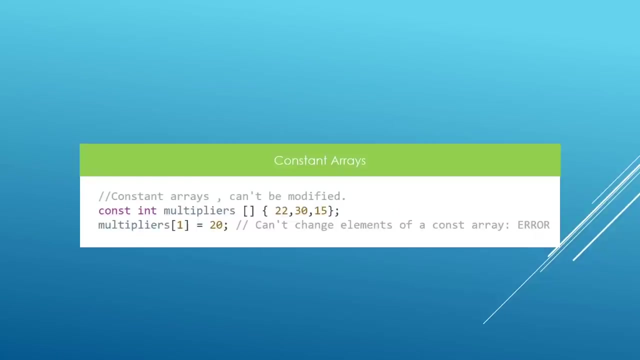 using a ranged base for a loop, because we don't have to set up an iterator, initialize it, do the test, do the implementation. we can just read the value and use it and be on our merry way. this is pretty cool. it is possible to also declare your array constant, and when you do that, 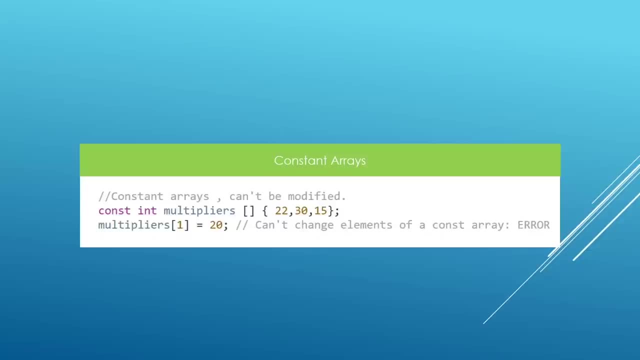 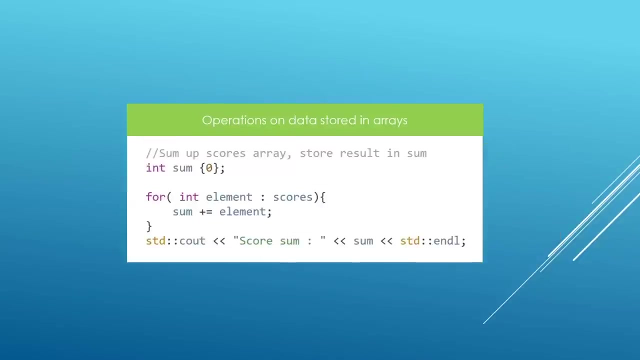 you won't be able to modify elements of that array. that's what it means. if you make it constant, you basically want it to stay constant and you don't want to allow modifications of your array. and we're going to see this in a minute when we get in visual studio code. the last thing i want you to see: 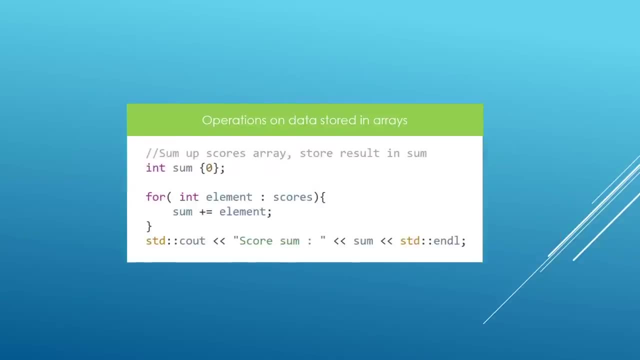 is that you can actually do operations on the data that you have stored in an array. for example, here you can see that the same type of array is stored in parallel and the same type of array is stored in parallel. so you can see that you can store the elements of that array if you want to store the. 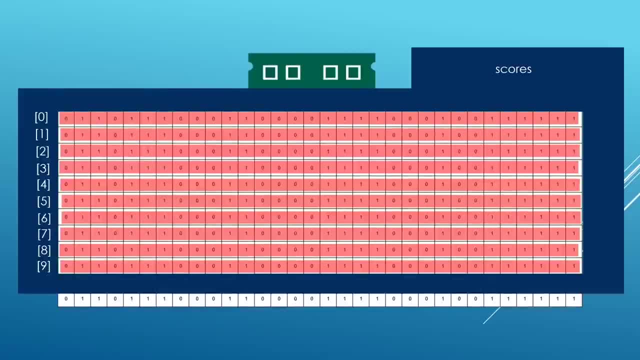 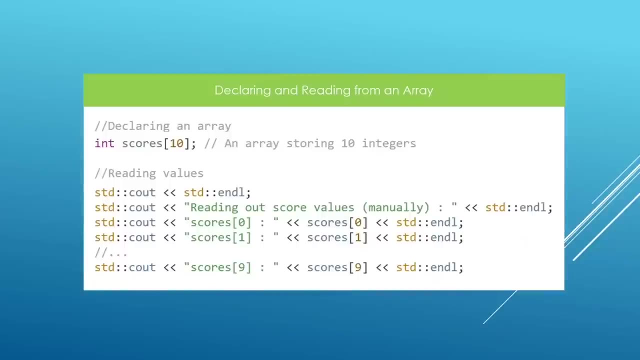 elements of that array and store the result back in our variable sum, and this is something you would do and it might come in handy in many times. okay, one thing i want you to see before we head over to visual studio code and play with us is that arrays store elements of the same type: repeat. 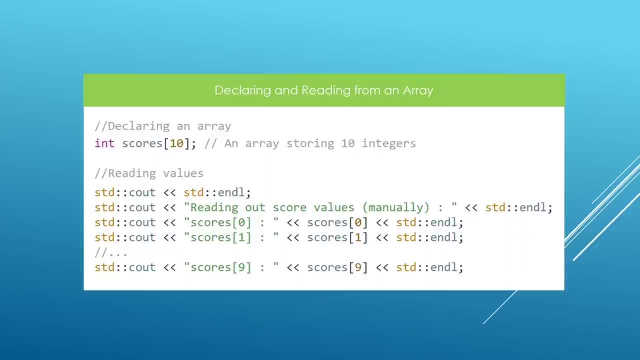 after me. arrays store elements of the same type, And if you try and store a different type than the type that was declared for the array, you're going to get a compiler error. So this is something you should keep in mind. but it makes sense, because when you declare an array, 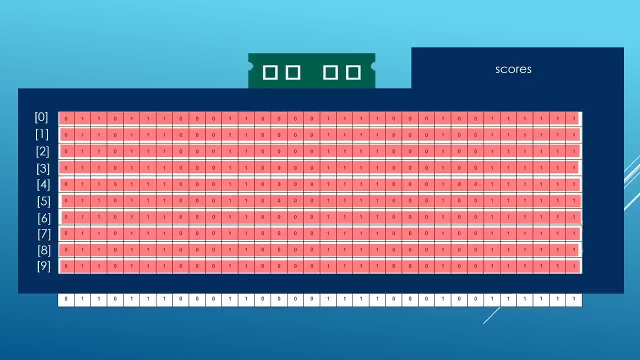 you're going to be given a bunch of bytes in memory and those bytes are going to be collections of data that is of the same type. For example, here we have a bunch of integers. Again, each of these rate events is an integer. 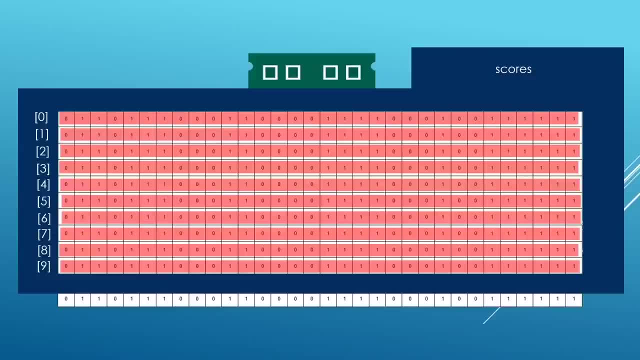 And if you try to put in something that is smaller or bigger than an int, then the compiler is going to be confused as to how to read these things. So for arrays to work, the types that you store in the array have to be the same. 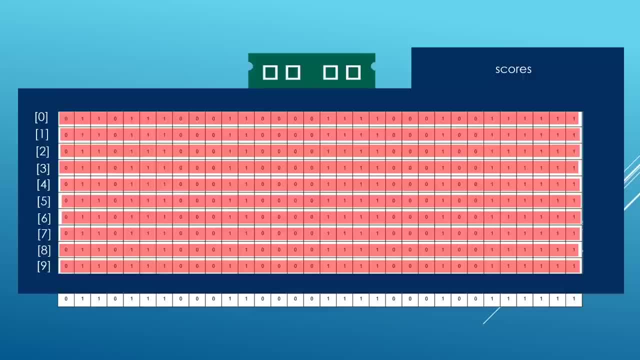 and they need to be consistent. This is something you should know, and if you try to break this rule, you're going to get a compiler error. Now that you know about arrays, we're going to head over to Visual Studio Code and play with them a little bit. 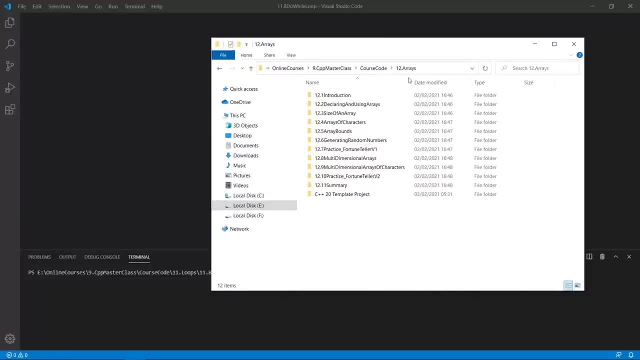 Okay, Here we are in our working folder. The current chapter is arrays. The current project is declaring and using arrays. We're going to grab our template code and we're going to copy and move the files over And we're going to open this thing up. 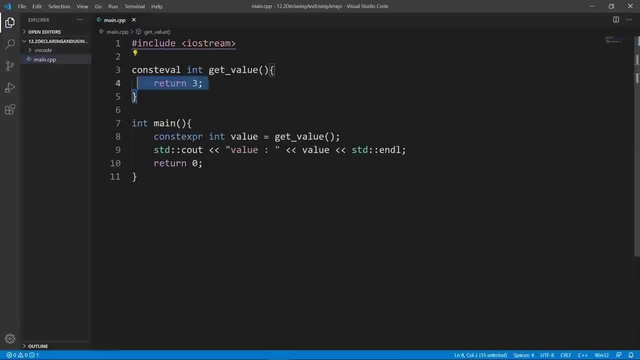 in Visual Studio Code pretty quick. We're going to open up the main CPP file and remove things we don't need, And we're going to see how we can declare an array of ints. Okay, We're going to do that. You say the name of the arrays. 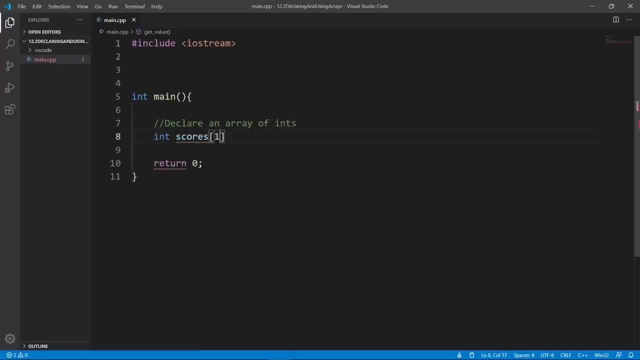 and you put this angle brackets and specify the size of your array. If you want, you can put a space in here, It's really not going to make a difference- And you're going to put a semicolon at the end The moment this line executes. 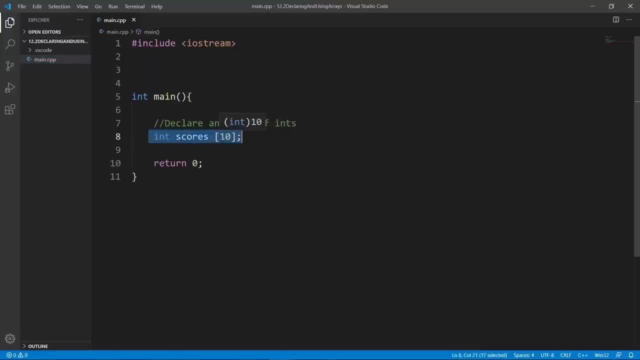 we're going to have the space for 10 integers allocated to us in memory, And that space is going to be called scores, And we're going to be able to read data from it or even write data back into it. For now, let's see how we can read the data. 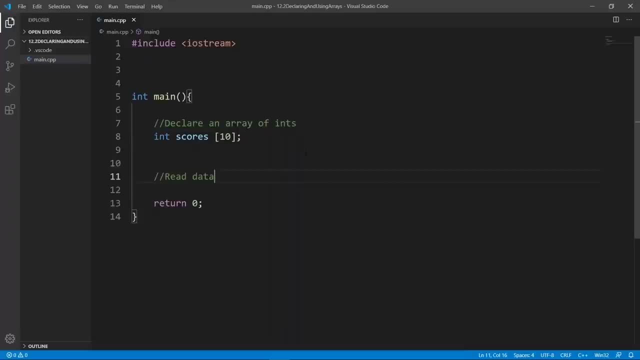 And it is really simple. We're going to use this angle brackets syntax that we just saw in the slides. So if we want to read the first element, we can say stdcout, We want to print it out And we're going to say scores. 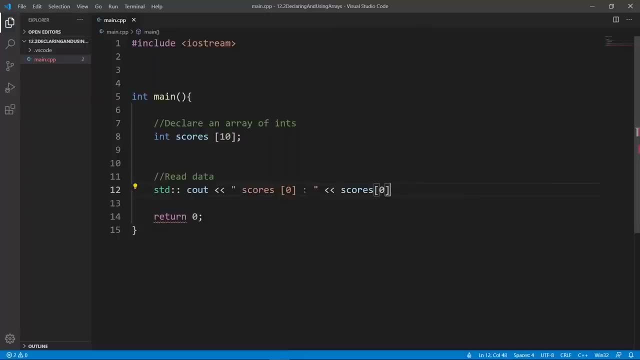 Specify the index we want to read from. So we say zero And we're going to say stdendl to move to the next line. If you have this typed out, you're going to see that this is going to work And it is going to print whatever is stored. 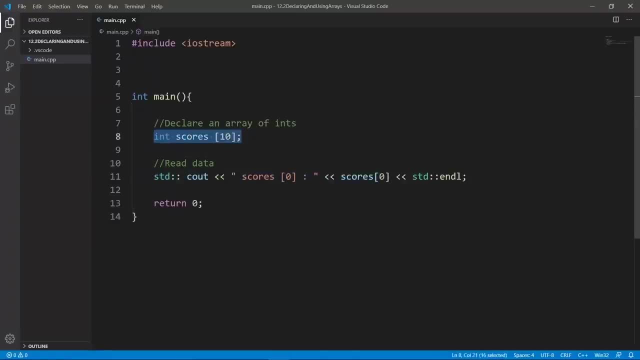 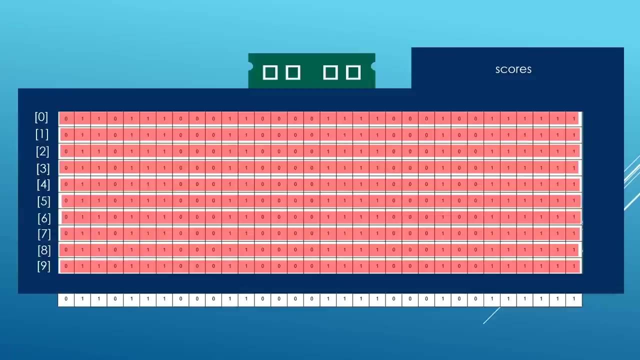 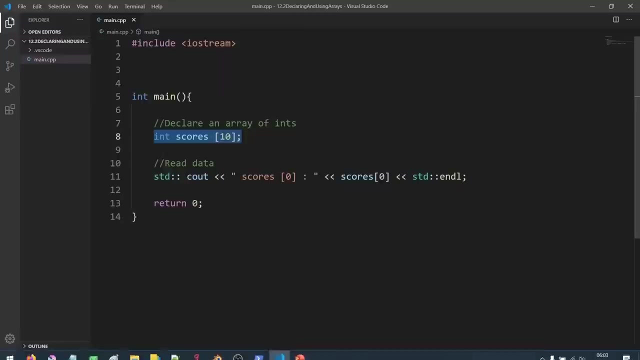 In the first element in this array. here And again, I want you to keep in mind the memory structure of your data when you are working with arrays. So what we're going to print right now is whatever junk data is in this first element here. 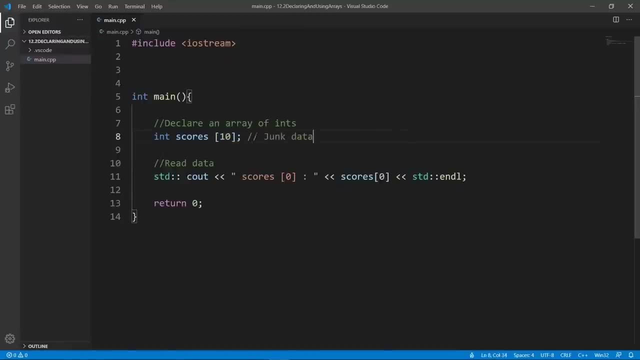 Okay, in here we're going to say that we have in junk data And let's bring up a terminal so that we can play with this. And we're going to build this with GCC, as we always do. The build is going to be good. 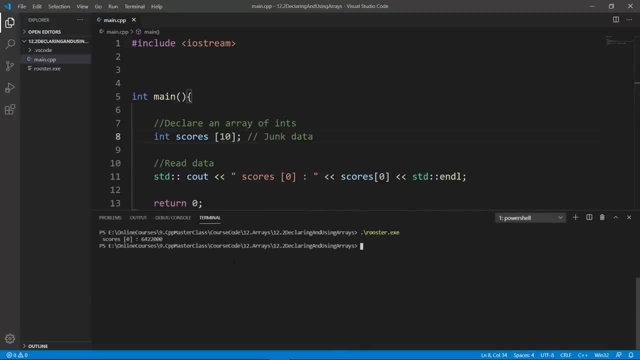 And we're going to clear and run rooster. You see that this is the junk value we have in here. We don't have any useful data in here. It's just junk data because we didn't initialize this array. We can also read the element at location too. 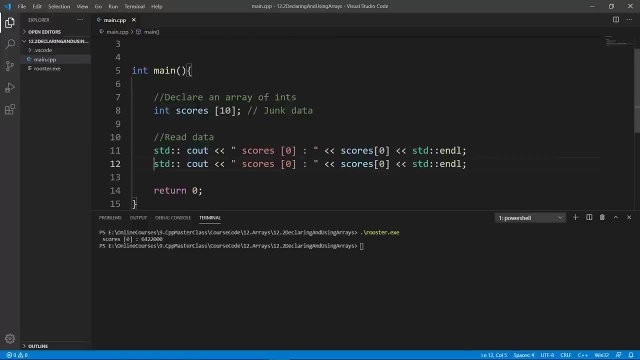 and see what we have in there when you run the program. I'm not even sure if it is guaranteed that you're going to get the same data if you run the program multiple times. But we don't really care, We know that it is junk data. 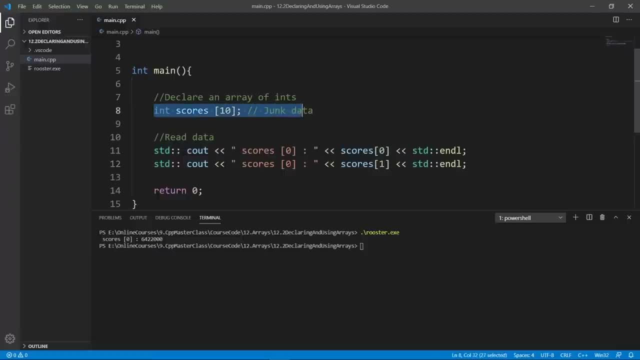 So we can't use this in our program. What we're going to do is run this and see the value for the element at index one. Let's build with GCC. The build is going to be good, We're going to clear and we're going to run rooster. 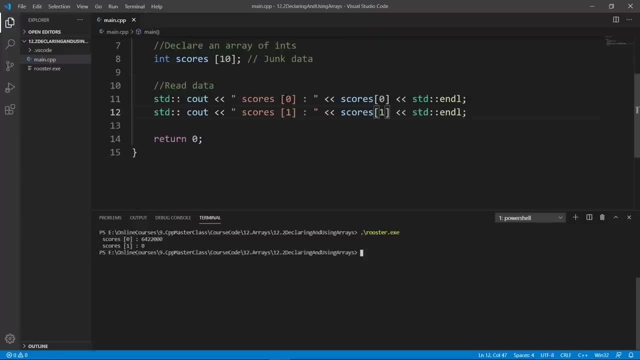 And you're going to see that at index one we have a zero end. But doing it manually like this is really time consuming And it is possible to actually do this in a loop. We know the size of this array, so it's a 10.. 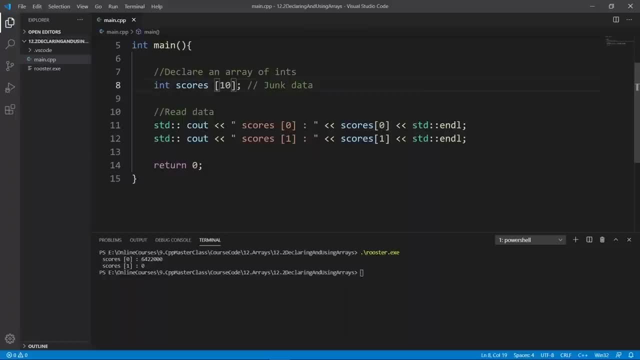 And we can loop around 10 times, creating each element at each iteration. And the way we do that, we're going to read with the loop and we're going to say: for okay, size t and we're going to start from index zero. 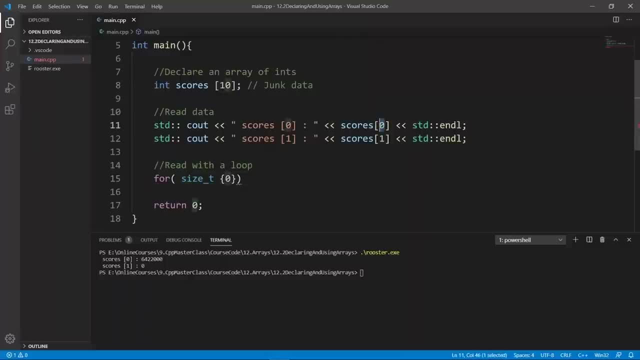 This is really important because arrays are indexed from zero. They don't start from one. Again, this is something you need to drill in your brain And we're going to put the index here. put in our test case, we're going to say i less than 10, because we want to go from 0 through 9. 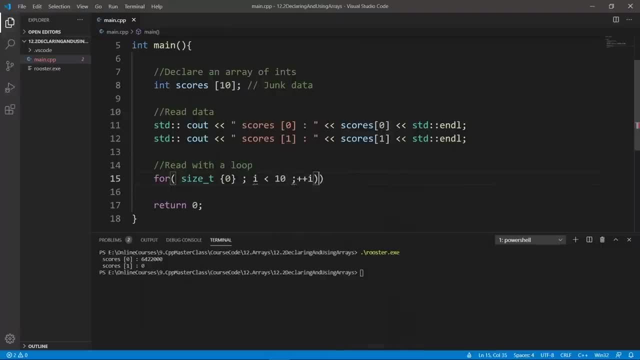 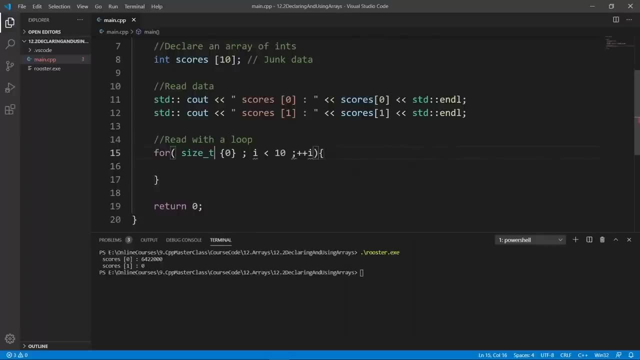 and we are going to increment our iterator. after we do that, we're going to have to jump into the body of the loop and we didn't name our iterator. that's why we have in this squiggly line here. let's do that pretty quick. we're going to jump into the body of our loop and we are going to 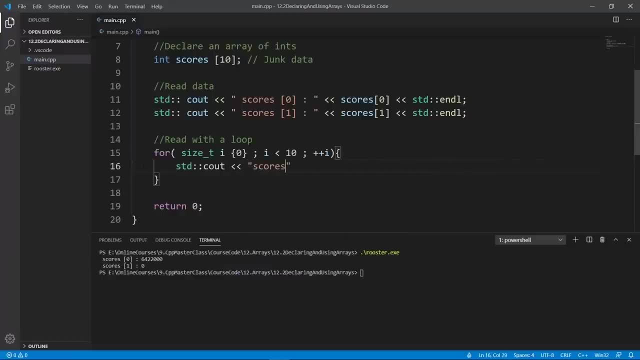 say stdc out and we're going to say scores. and we need to be careful about how we format this because i is not something we have. we're going to be getting that from our iterator here, so we're going to print it like this and this is going to work no big deal. and we're going to say scores. 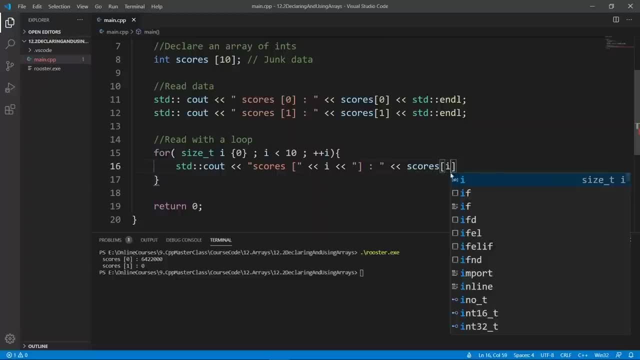 and we're going to say i, that's going to be our index, that we want to print the data for, and we're going to say stdendl and, and, and. because we don't want this to confuse us, we're going to comment that out and we're going to 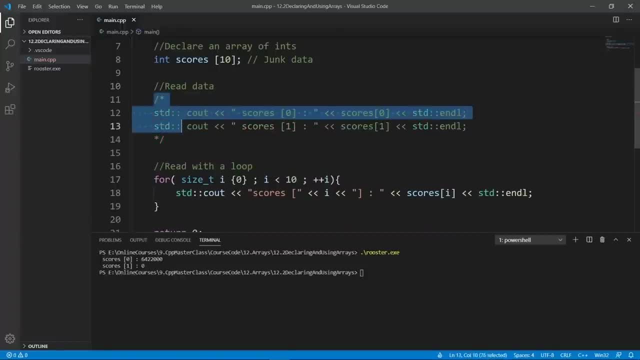 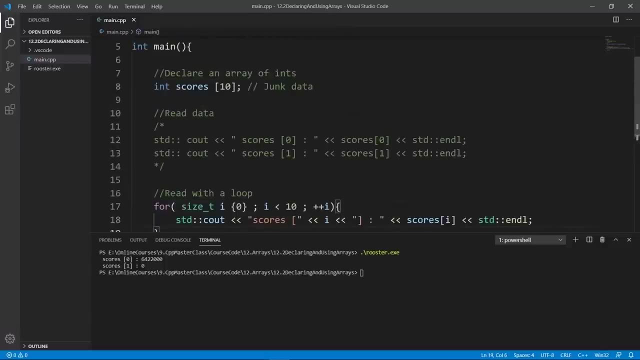 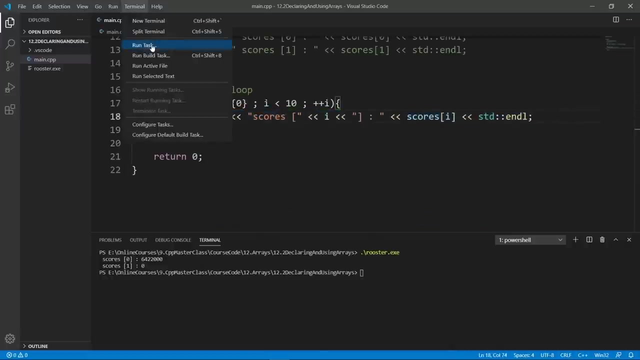 go up and make sure our comment is nice and neat, and we're going to try and run this. and what do you expect to see? well, we don't have any real data in here. we're going to have some junk data, so it could really be anything we get printed here. so let's world with gcc and we're going to 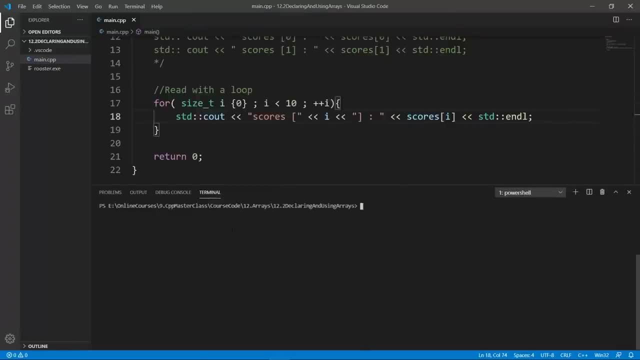 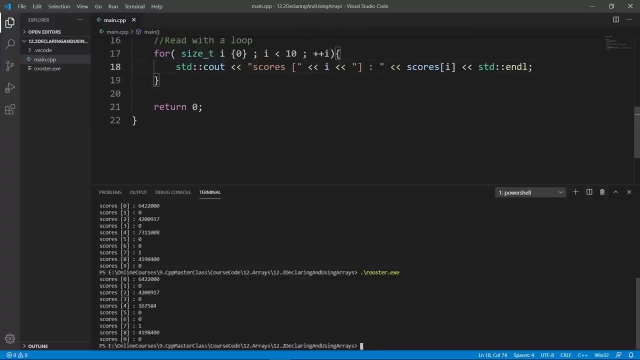 give ourselves some breathing room. we're going to go down and clear and run rooster and you see that, hmm, this is really some junk data. and if we run it again, let's see that we get the same output. it is the same data in here. if we want to have in some reliable data, we need to write in our 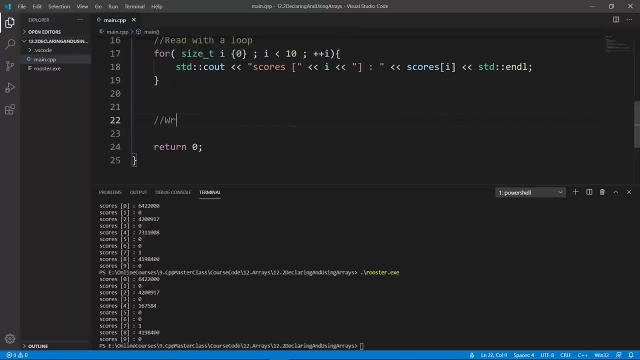 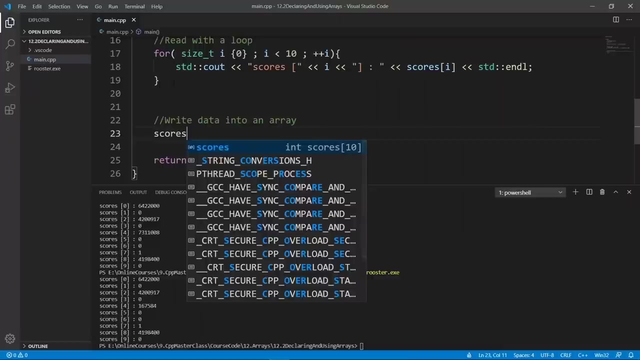 own data and we're going to see how we can do that. we're going to see how we can write data into an array and the syntax is really simple. so the way you do that a, you just say the index for which you want to write data in, and you say scores and you specify. 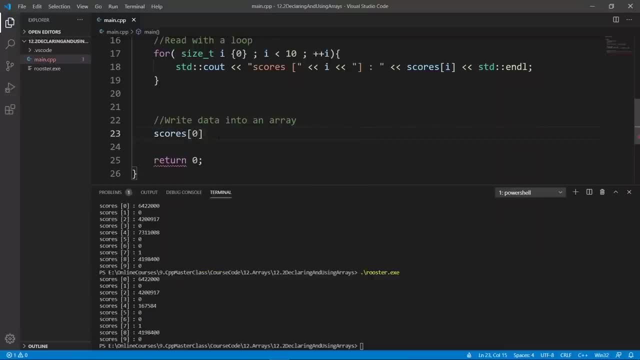 the index. let's say zero, and we're going to put in a 20, for example. this is how you do this: you say 20, let's say scores. we're going to grab the index one, the first element, and we're going to put in a 21- why not? and we're going to say scores. we're going to say 2 for index 2 and we're going. 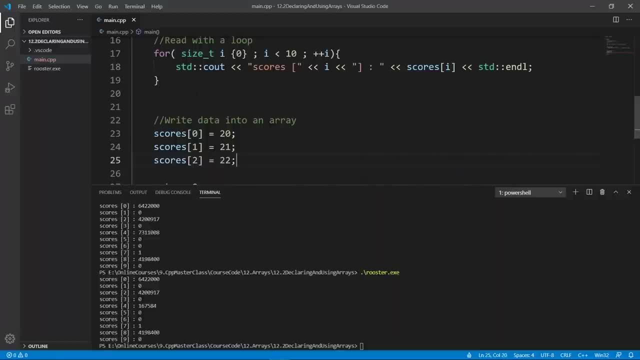 to put in 22, why not? and after we do this, we can print this out or read data with the loop and make sure that the data we did write in is actually in. so we're going to copy this and comment this out, because we don't want this to confuse us on the console, and we're going to do that. we're going to 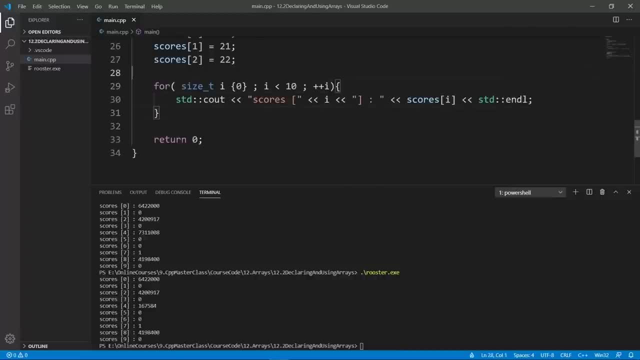 come down here and print the data out. let's say what we're doing here and if we build this, we expect to see that you index 0, 1 and 2. we have the values 20, 21 and 22. let's build and see. we're going to run the test. 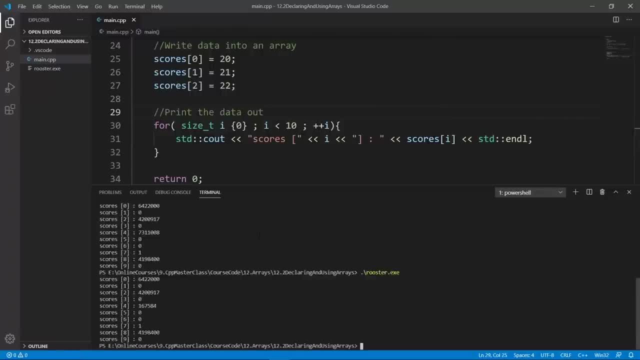 to build with gcc. the build is going to go through. we're going to clear and run rooster and look at this: scores 0, 20 scores 1, 21, scores 2: 22 and our data is actually getting in. now we're going to. 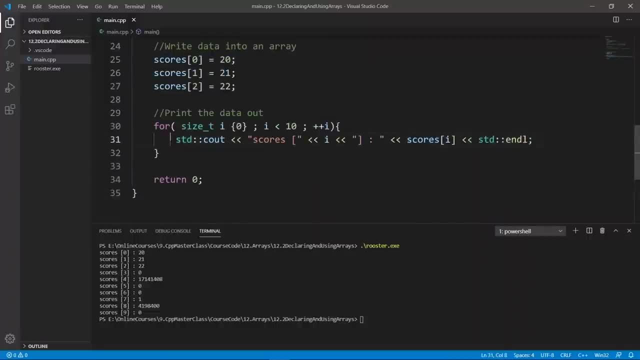 see that we can also write the data using the loop to make it really easy without us manually doing things like this. for that, we're going to copy what we have here to print data out and we're going to comment what we had out here. so let's comment this out and we're going to go. 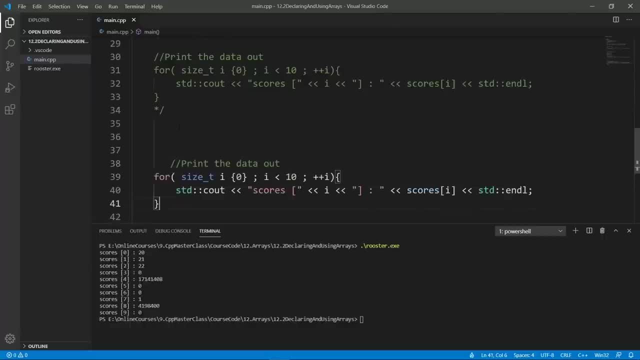 down and print the data again. we're going to put in the code here and before we print the data, we're going to put data in with a loop. so the loop is basically going to be the same thing. we're going to say size ti. we're going to initialize this. we're going to say i list done. 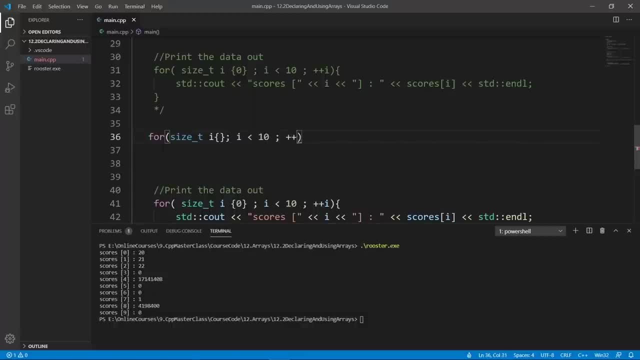 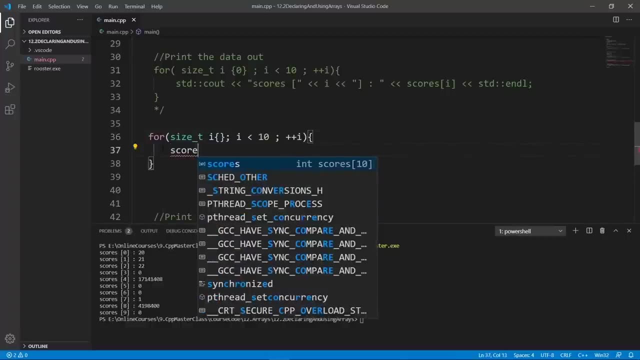 10 because we want to loop 10 times. we're going to increment and we're going to fall in the body of the loop. what we're going to do is write data at the index of the current iteration. i should say so. what we're going to do, we're going to say scores i and we can really put in anything for 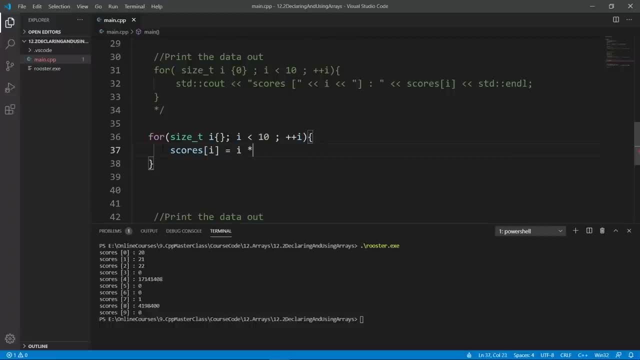 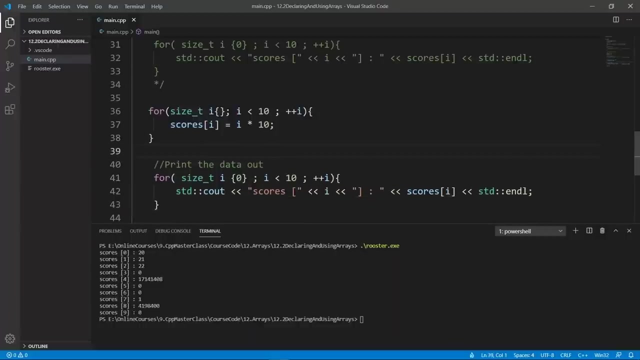 now let's say we want to put an i multiplied by 10.. so we're going to take the current index, multiply it by 10 and we're going to store that in the index. at the current iteration. this is what we are doing here and if we print this out, try to think about what we're going to get here. 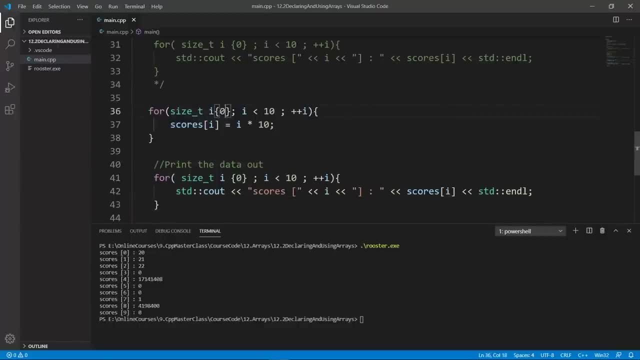 so at index 0 let's put in a 0. to be super clear here that we are starting from index 0. at index 0 we're going to take 0 and multiply that with a 10, so we're going to store 0 at index 0.. the loop is: 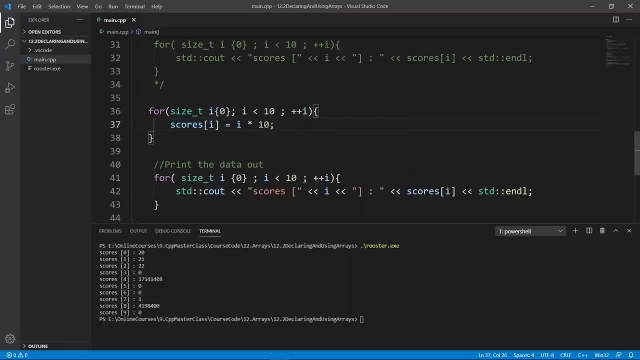 going to run again at index 1. we're going to take a 1, multiply with 10, we're going to get a 10. at index 2, we're going to multiply 2 with a 10 and store a 20 at index 2 and we're going to keep going and basically have 0, 10, 20 all the way to 90 stored. 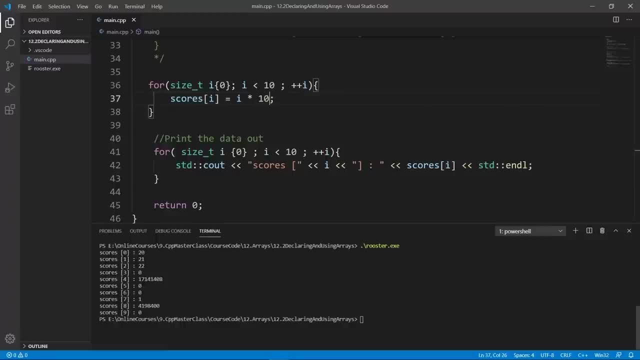 in our array here. so if we print it out we expect to see 0, 10, 20, all the way to 90.. let's weld and see that that's actually what we have in our array. we're going to work successfully. let's clear and run rooster and you see that this is exactly the same thing we have in our array. how? 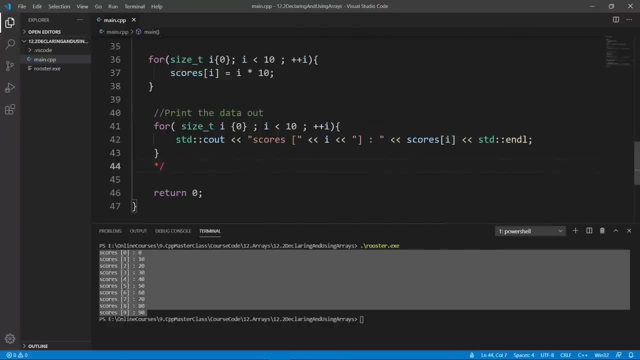 cool, is that okay? another thing i want you to see is that we can declare and initialize an array in place, but before we do that, let's say what we were doing here. we were trying to write data in a loop, and we're going to comment this out because we don't want a lot of 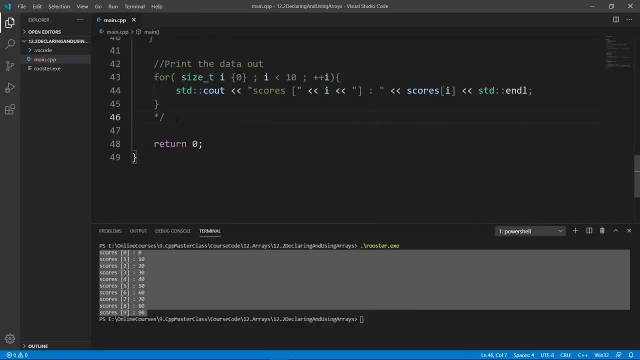 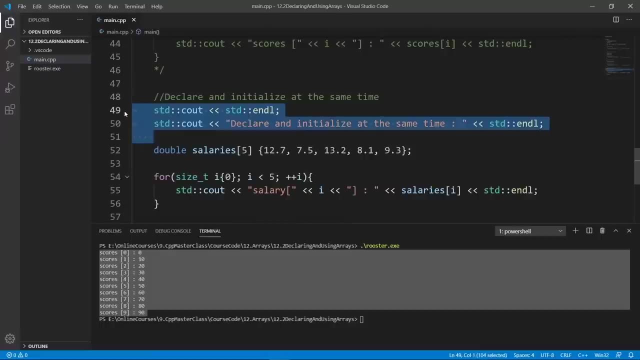 confusing output in our console and we're going to go down and put in the data- because i don't want to type all these things- so we can declare and initialize an array in place and the way we do that, the array is going to store doubles. now we can really declare an array. 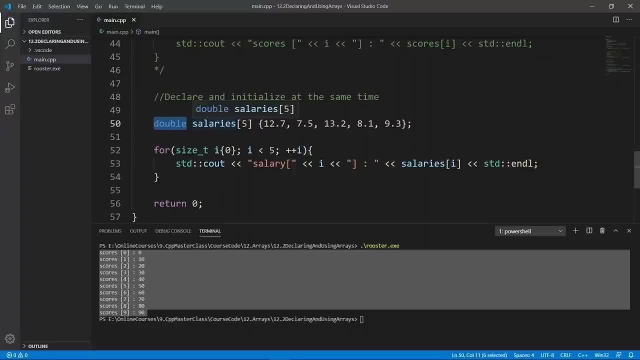 of anything, but so far we have seen that we can do that for- and now let's try a little bit and show you that you can do the same thing for double types. so we can declare an array of double types. the size is going to be 5 and we're going to initialize that with this data here, so at index. 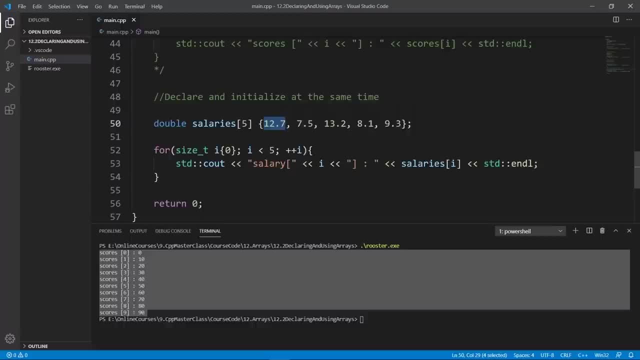 0. we're going to have a 12.7 index 1 is 7.5, index 2, a 13.2, index 3 and 8.1 and index 4 and 9.3. and that's what we're going to have if we print this out here. we have a simple loop to print it out and 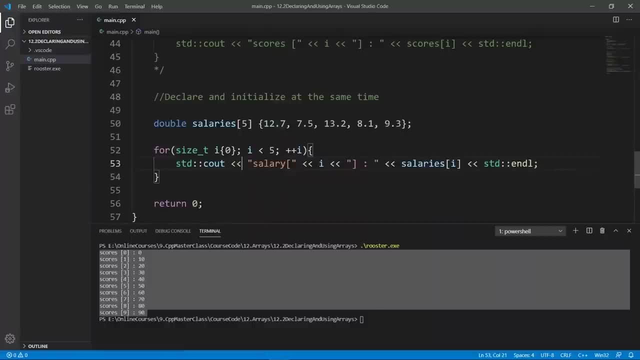 it's going to basically say salary 0- 12.7, and it's going to go all the way to salary 4 and print a 9.3, and this is something you can do if it makes sense for whatever you are designing with c plus plus. 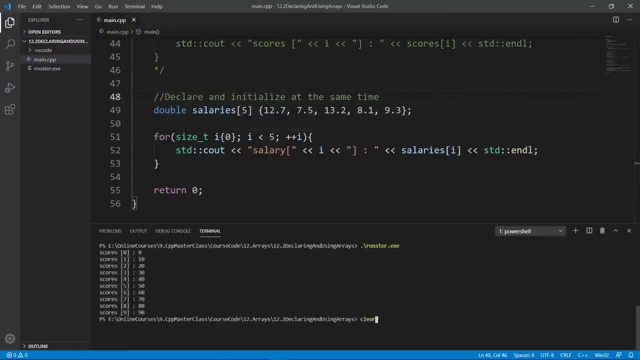 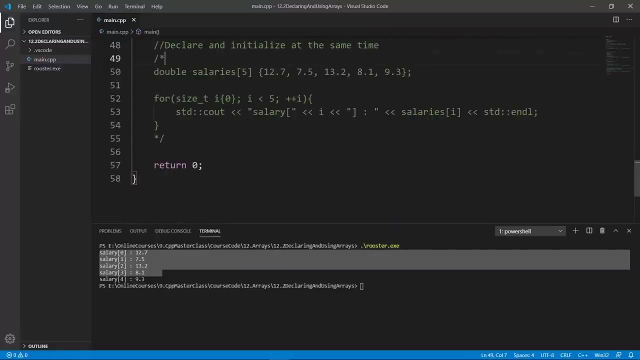 we're going to build this with gcc. let's clear and run, and you see that this is exactly what we expect. okay, now this is super clear. the next thing we're going to see is that if you don't initialize all the elements in the array, those you leave out are going to be initialized to zero and we are going to put in a piece of code to: 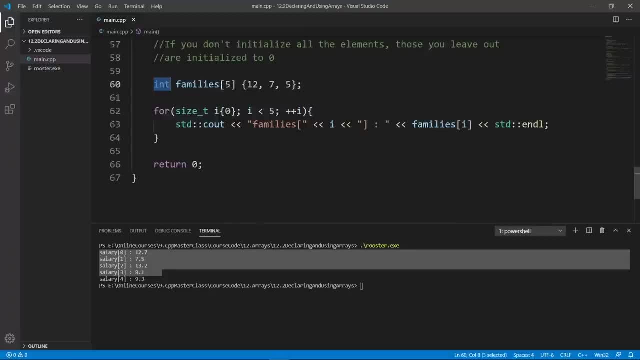 play with that. so here we have an array. it's a net array, it's going to be called families and the size is going to be five. but we are only initializing three elements and these elements are going to be elements on the front, so elements at index three and four. 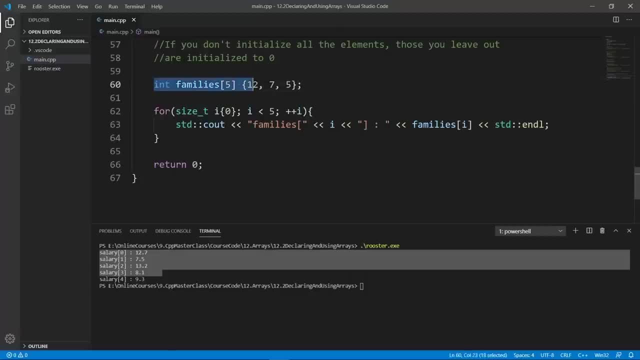 are going to be left out and they are going to be initialized to zero by the compiler. so if we print this out, we expect to get 12, 7, 5 and 0, 0 at different indexes in this array here. let's build this with gcc. we're going to clear because the build is successful and we're going to run this. 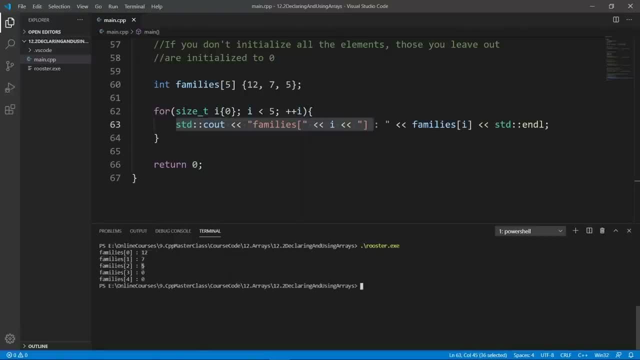 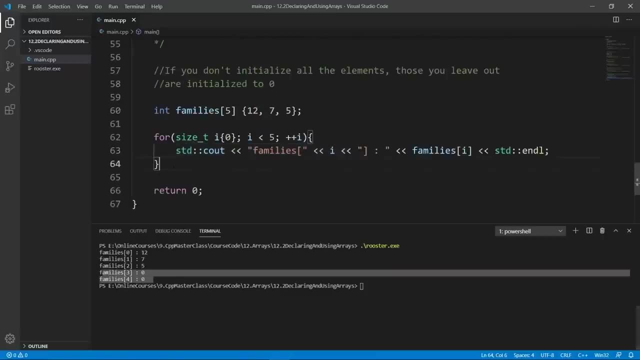 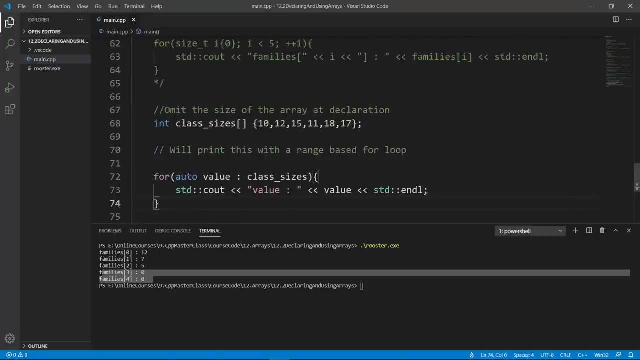 this is exactly what we expect. we have a 12, a 7, a 5, and the last two elements are initialized to 0, and this may come in handy sometimes. okay, let's comment this out. another thing we want to see is that we can actually omit the size when we are declaring our array and initializing it. 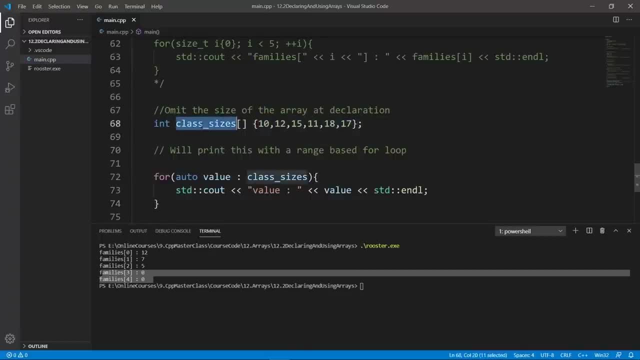 so here is a simple example. we have an inter-ray called class sizes. we don't specify the size, but we initialize it and the compiler is going to deduce the size of this array from the elements we put in here. so if we put in two elements, so it's going to be of size 2. if we put in 10 elements, it's going to be of size 10. 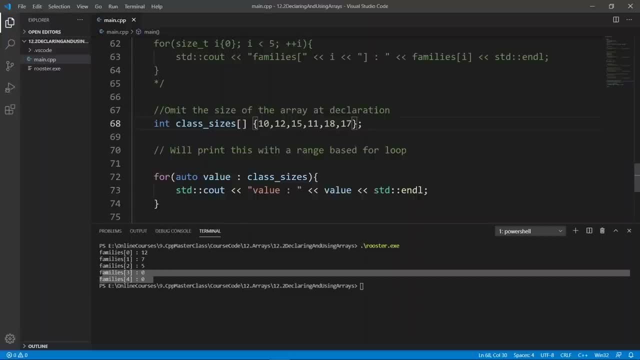 and this is how this works. but if you do something like this and not initialize the array- let's take this out for example- you're going to get a compiler error because the compiler now doesn't know which size it's going to give to this array. so be sure to either. 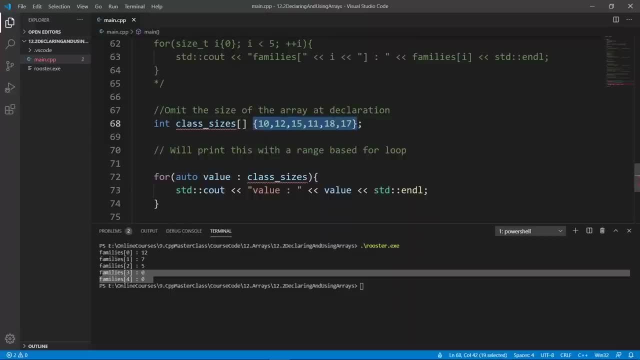 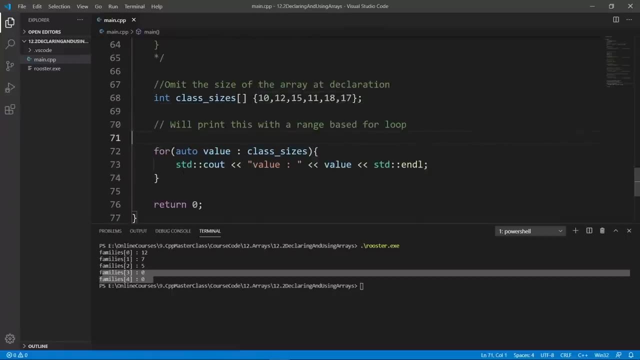 put in the size or initialize your array like this, and it is going to work. this case we're going to have six elements in and you see that a range based for loop is going to come in handy here, because we don't really know the size of this array if somebody comes and adds. 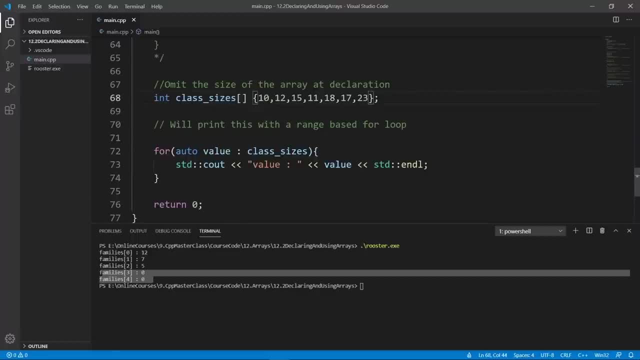 in another element, let's say 23, the size is going to change and if we hard code the size in our full loop, the code is going to break. but a range based for loop is going to use whatever size this array has. so we're going to try and build this. we're going to build with gcc, as usual. 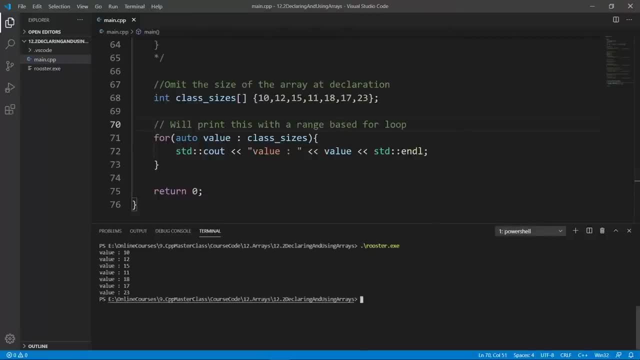 and the world is going to go through. if we run rooster, we're going to get the elements we have: 10, 12, 15, 11, 18, 17, 23. if we add a new element, this is going to work. you see that we don't. 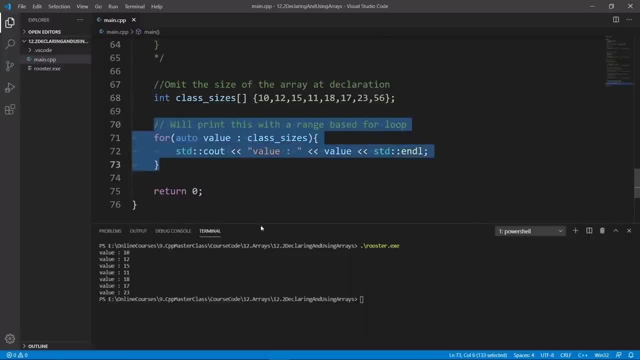 need to modify the loop here to put in the new size, and this is really cool. i like this about range based for loop. so we're going to build again and we're going to clear run rooster and this is going to give us exactly the data we have in the array. so this is one way you can. 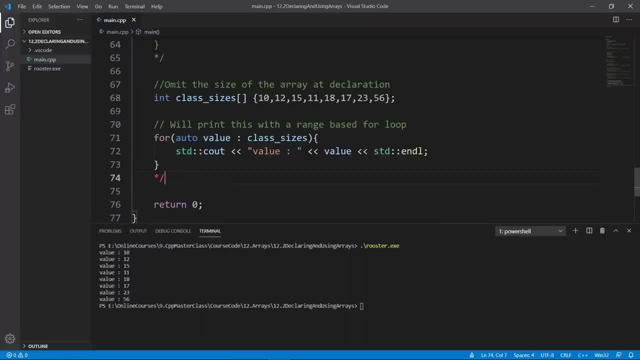 do things. another thing we saw is that you can't modify cost arrays. so let's do an example here. for example, we're going to grab this thing and put an array declared down here, we're going to copy that and use that here and we're going to make this cost. let's give it a name, let's say birds for. 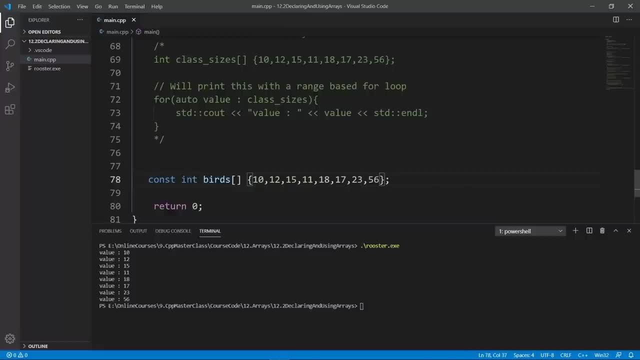 example. for example, we want to keep track of lines of birds or whatever. this is just an example to you that you can't modify this array. so if you're trying to do something like birds and index 2, for example, and you want to change this to an 8, the compiler is going to complain. you see that visual. 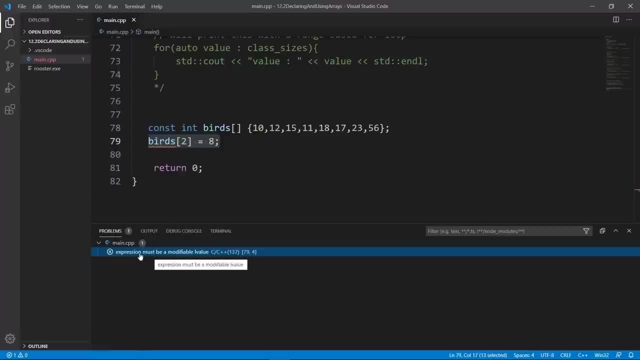 studio code is complaining already: expiration must be a modifiable value. so it is saying that the array stores const elements. so you can't modify elements of this array. okay, so this is something you can do. if you don't want to modify the array, you can do this. so we're going to do this. 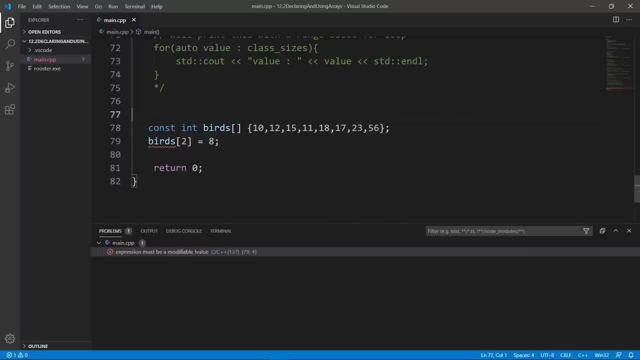 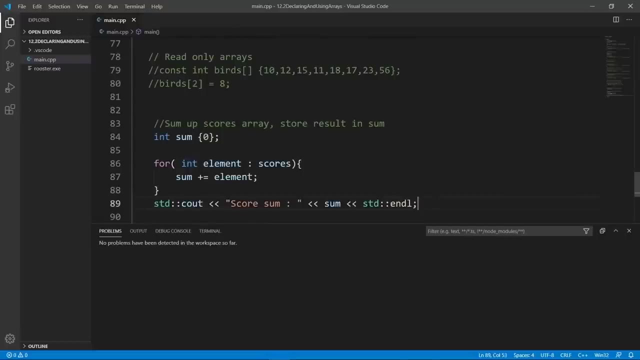 don't want people to be able to modify data in your array, and the last thing i'm going to show you is that you can do operations on the data in an array. so let's bring up our scores array again. so we're going to go up and copy it because the code is using it. so let's put in our own scores. 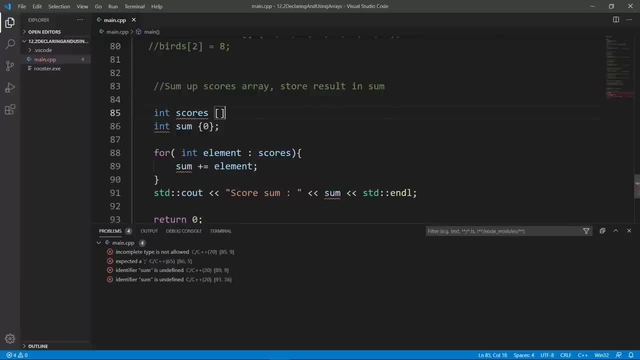 array. it's going to be pretty fast and we're going to say that it is an array with this angle brackets. we're going to initialize this. let's put in a bunch of values and what we can do is sum these things up. we're going to store our result in the sum variable and we're going to loop around. 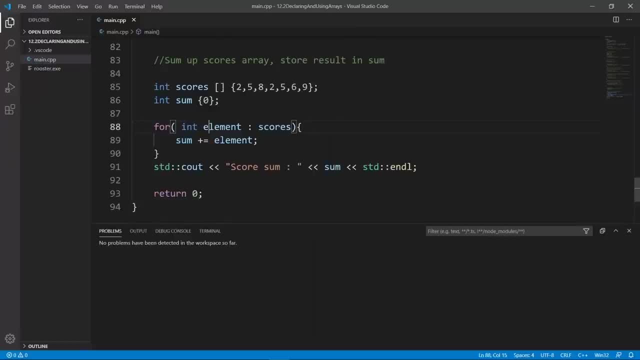 with a ranged based for loop because we don't really know the size of this array. it can change any time, with however many elements, and a ranged based for loop is really cool in that we don't have to keep track of the size ourselves, so we're going to go in here and get each 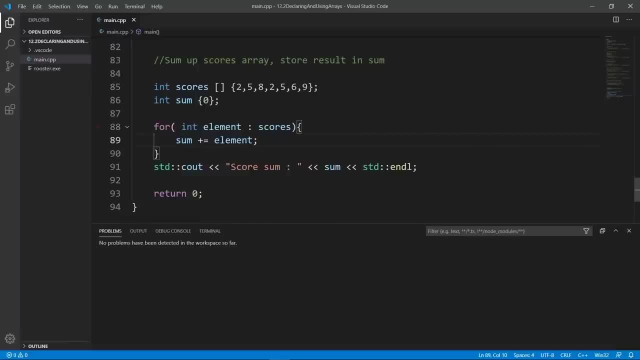 element and we're going to go in here and get each element and we're going to go in here and add that to sum. so, for example, for the first time, sum is going to be zero, because that's what we initialize it with. we're going to get into this loop here. the first element is going to be two. 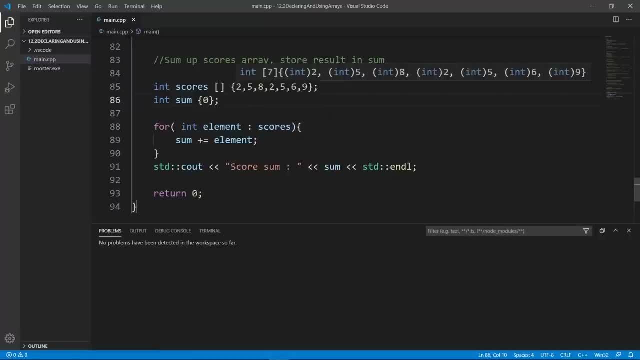 we're going to add that to zero and get two. we're going to add a five, we're going to get a seven. we're going to keep adding these elements and, at the end, sum is going to contain the sum of all these elements in the array here, and this is one cool way you can sum up the elements in your array. 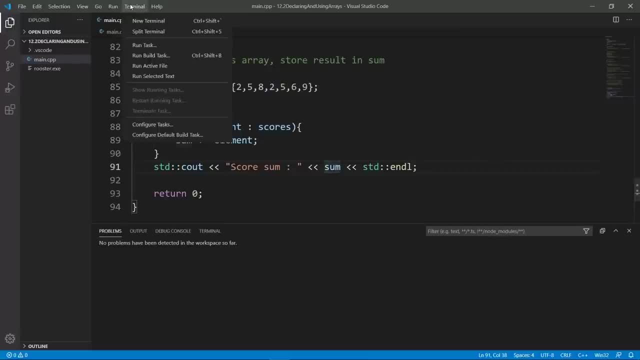 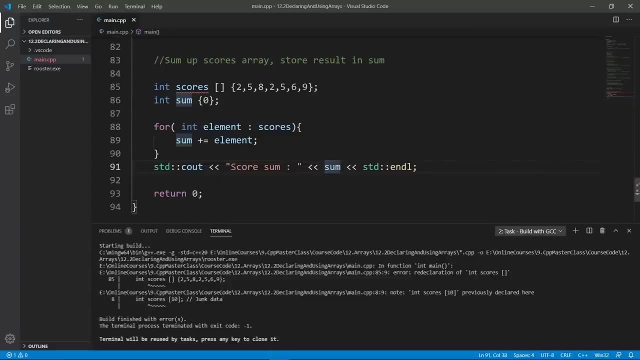 so if we run this, we're going to get the sum printed out. let's do that pretty quick. we're going to run the task to build with gcc and we have ourselves a compiler error. what is happening here? it's going to say redeclaration of scores. where did we declare scores before? let's go up. 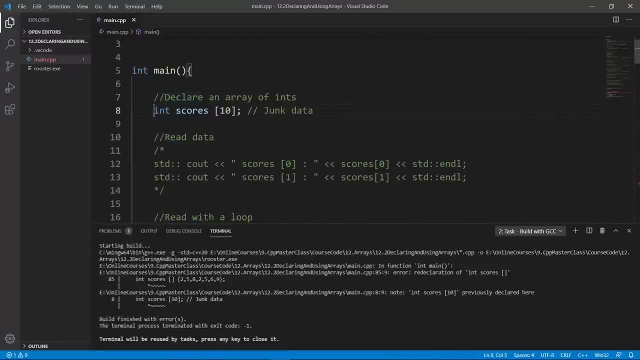 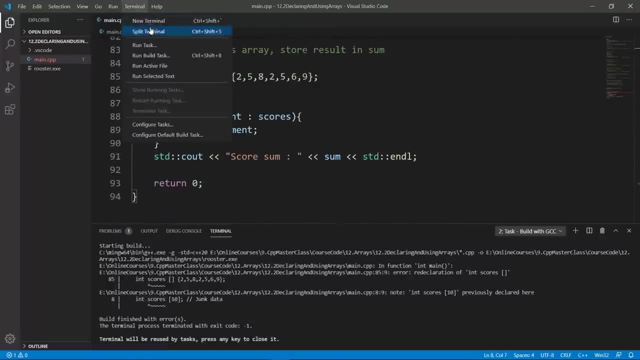 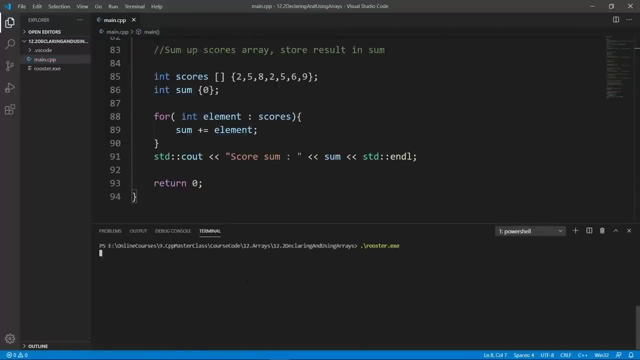 and make sure it is not declared somewhere. and it is declared here. so we want to comment this out, come back to our code so that we can see it, and we're going to build again and we're going to run it again with gcc, and now the world is going through, we're going to clear and if we run rooster- 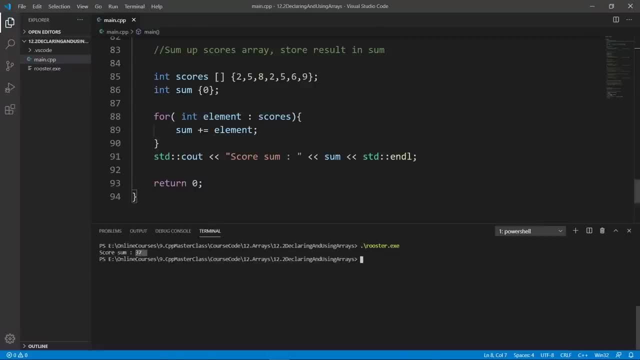 score sum is 37 and if you sum these things up, i'm sure you get a 37.. this is really all we set out to do in this lecture. i hope you have a better idea of how you can declare your arrays, put data in, read data out of those arrays, make them const or even do all kinds of operations on them, and 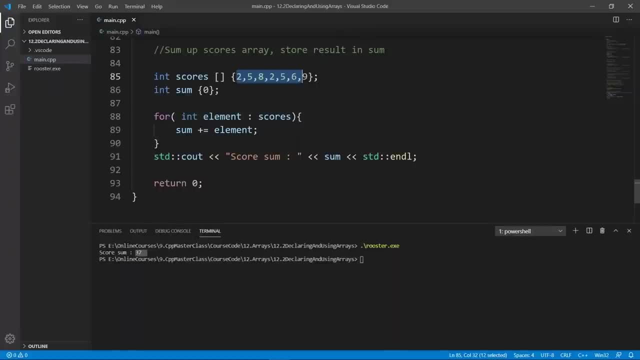 this was really what this lecture was about. we are going to stop here in this lecture. in the next one we're going to see a cool way we can use to get the size of an array. go ahead and finish up here and meet me there. in this lecture we're 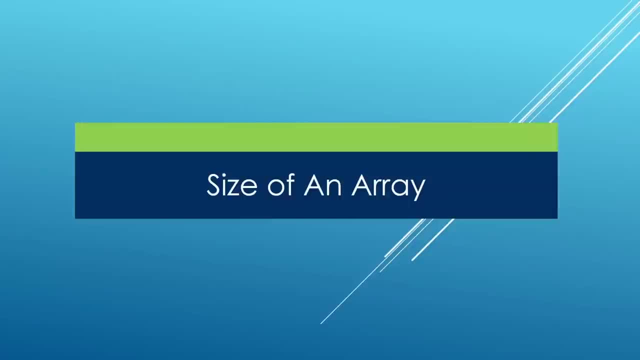 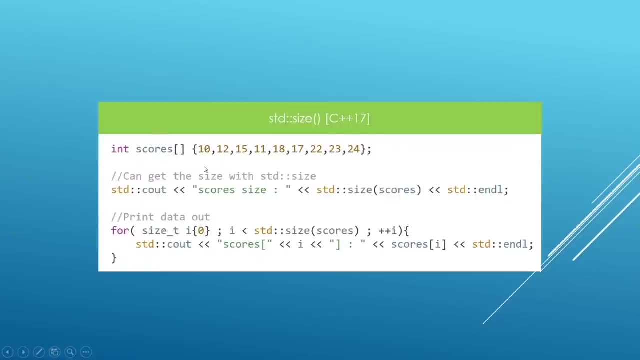 going to see a way we can query for the size of an array at runtime. if you remember, in the last lecture we had an example like this showing how we can declare an array and initialize it in a single statement like this. but the problem we had with this is that 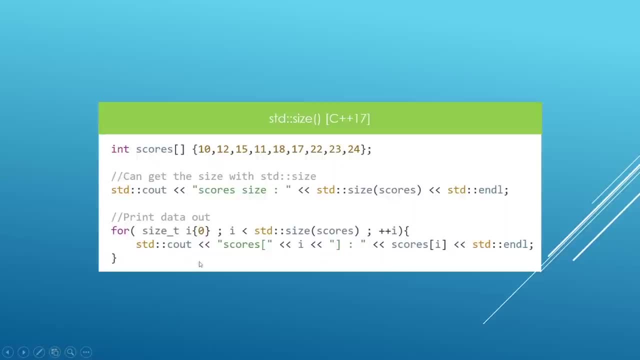 if we tried to print the array using a for loop, for example, we would have to use the size, and the size of this array may change if somebody decides to add elements or remove elements. then the size is going to be irrelevant. c++ provides a way we can query for the size of an array at runtime. 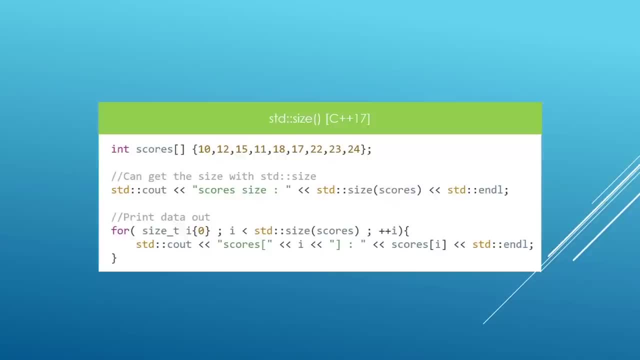 and we're going to get the real size accounting for the current number of elements that we have in the array, and for that we use the std size function. this is a function that comes with the c++ standard library, so you're going to have it already if you have a compliant compiler. if you see here, you see that it was introduced in c++ 17. 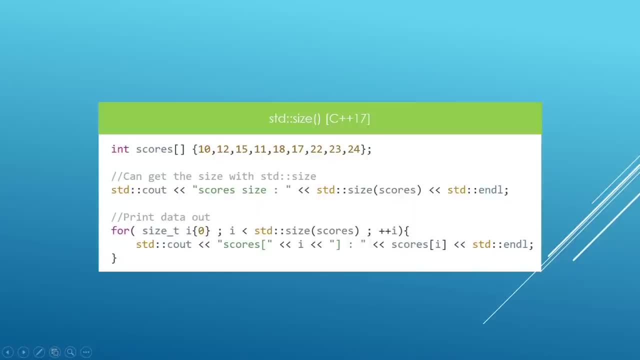 and it is a cool addition. we can use it to make our code easier to work with. if you look here, we have a simple loop which is going to print data out. it is going to loop starting from zero all the way to the size of the array. you see that we use this to control when this loop is going to end. 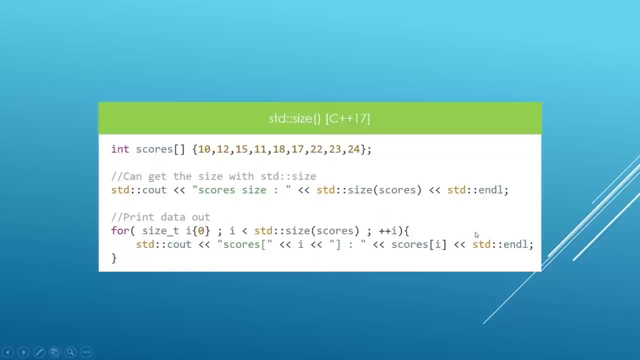 in our incrementation part and then we jump into the body of the loop and print the current element in the loop and if we do things like this, we're going to be able to print all elements in the array, regardless of the number we initialize it with. okay, so this is one way and it was introduced. 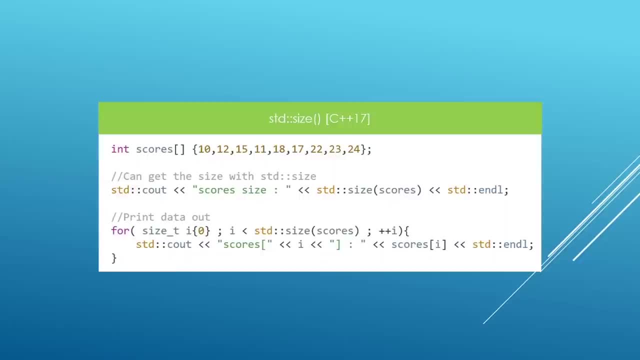 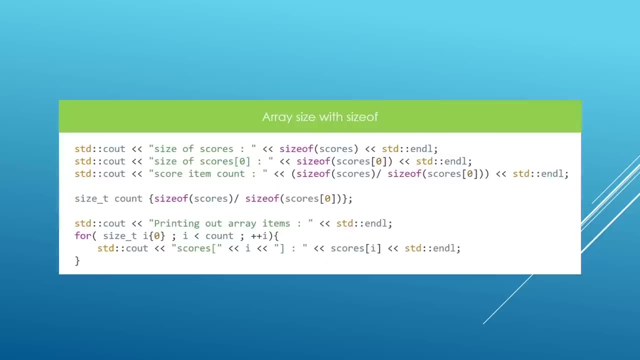 in c++ 17.. but some of you must be asking: how did we do things before c++ 17? well, we had to kind of do a hack to get something like this. we used the c++ standard library and we used the size of operator. we have seen a lot of times right now and the way you use this, if you do. 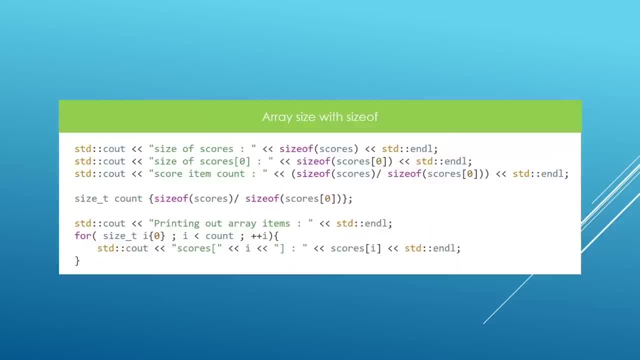 size of and pass in the array, you're going to get the entire size of the array. so if we take that and divide that with the size of a single element in the array, we're going to get the number of elements of the array. and this is really what we are doing here. we are setting up a count variable. 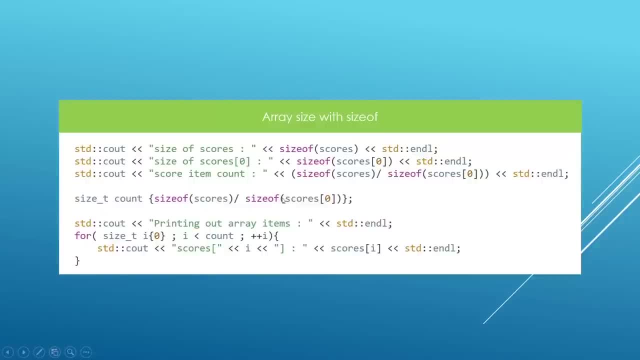 and we are taking the size of the array and dividing that with the size of a single element in the array and we are just grabbing the first element, because you can really use any element here and once we have this, we can use this count to do a loop like this and 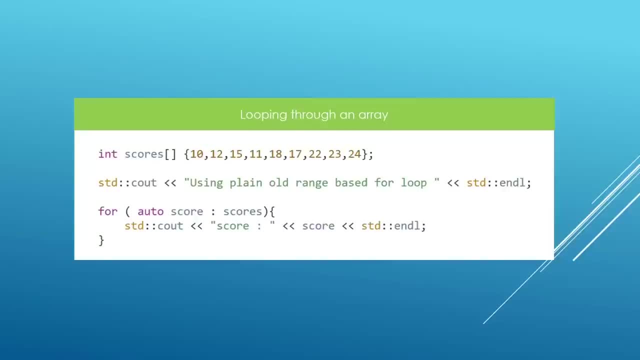 it is working pretty well. please remember that you don't have to go through this craziness we're doing here. you don't even have to use std size because you can use a ranged base for loop and get access to the elements you have in the array, and it is going to work pretty well now that you. 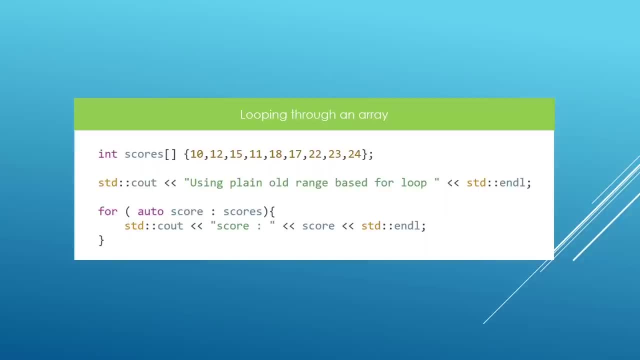 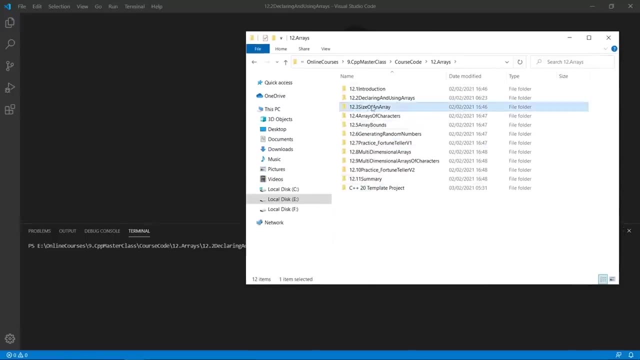 have an idea about this. let's head to visual studio code and actually play with this. okay, so here we are in our working folder. we are going to be working on this project size of an array. we're going to grab our template project. we're going to copy the files and put them in place. 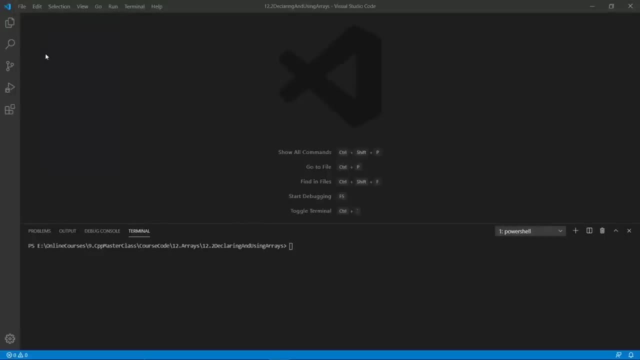 and we're going to open this up in visual studio code. let's do that. it's going to open up in visual studio code and we're going to try and clean it up a little bit. and we are going to declare an array and we're going to put in our name. so let's put in our name and we're going to. 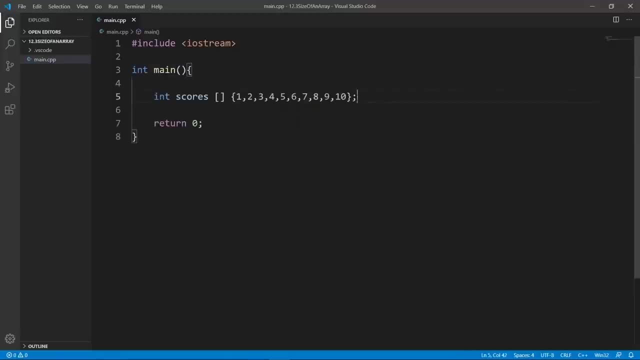 array. if we want to print this thing, we need to know how many times we're going to loop and print elements in here. so one thing you might want to do is to say: okay, we have 10 elements in here, so i'm going to loop for 10 times. you might think this is going to work, and it is going to work. 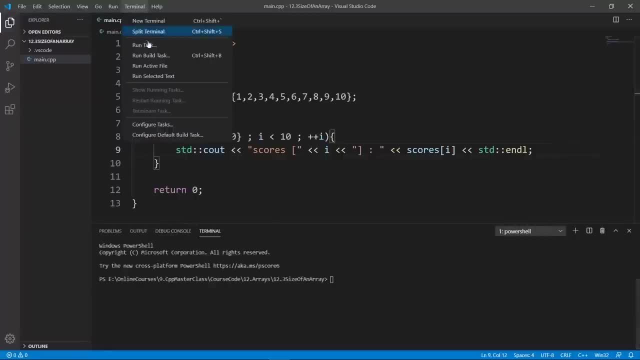 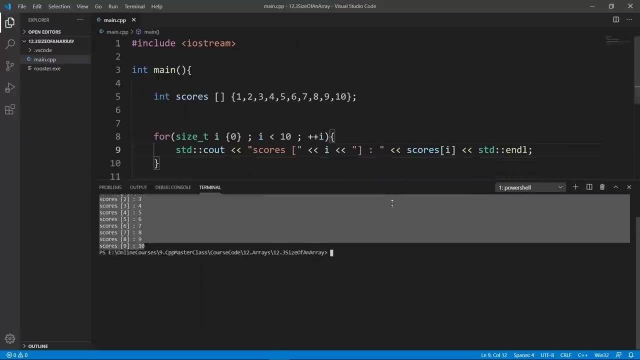 if we bring up a terminal and work this with gcc like we usually do and clear and run rooster, we are going to get our numbers. this is what we have in the array from 1 to 10. but what if somebody comes and changes the elements we have in here? let's add an 11. 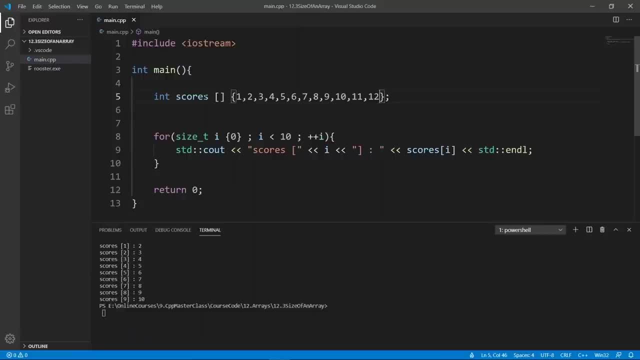 and a 12, and the moment we change this, we will need to come and change the size in here, and this loop here might be buried somewhere deep in your project and it might not be as easy as it is now to see that we, you, you- also need to change this. this may be a really big source of hard to debug problems. so what we? 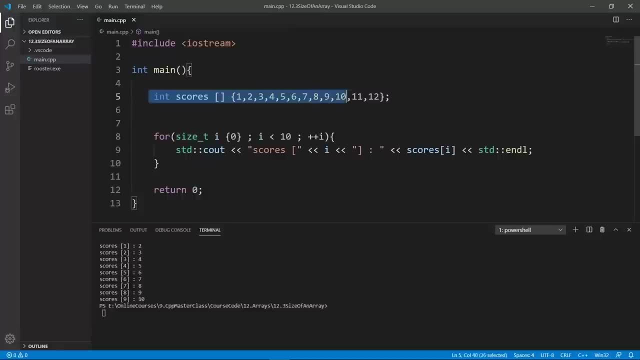 really need is a way to get the size of the array at run time and be able to dynamically query for that size and use it in our program. and that's exactly what std size provides. so we're going to say int count and we're going to put in a value. let's use a braced initializer, so we're going to 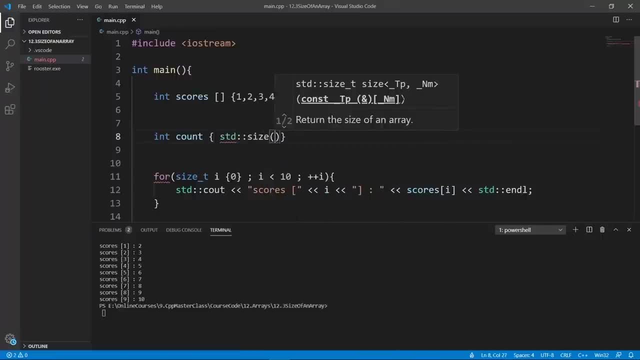 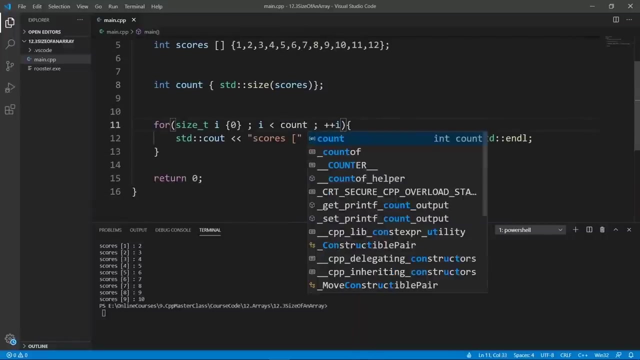 say std size, and we're going to pass the array we want to get the size for and if we do this, we're going to get this size here and we're going to be looping for this number of times. so we're going to test, for i is less than count here and now it doesn't. 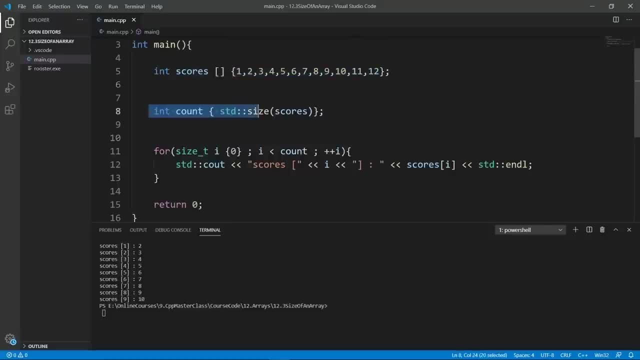 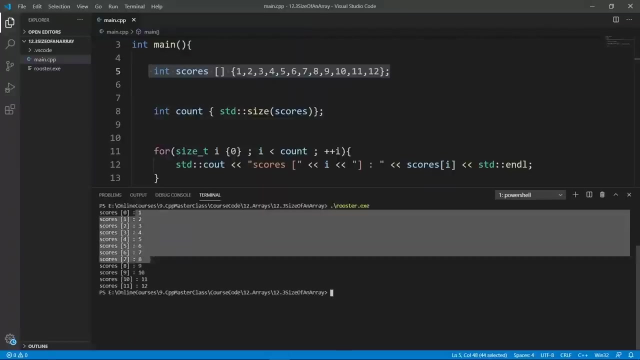 matter how many elements we have in here, we're going to get them at run time. we need to only update this initializer here. so what we can do is weld with gcc again. now we're going to come here and run rooster and we're going to get the numbers here. you see that we get. 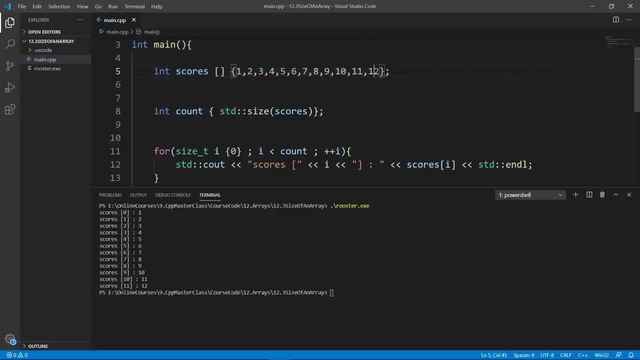 the elements. if we take out a few of these elements. let's take out a few of these, let's leave in up to seven or eight, let's build again and we are going to clear and run rooster. we're going to get however many elements we have in there and this is pretty cool again, you might ask. 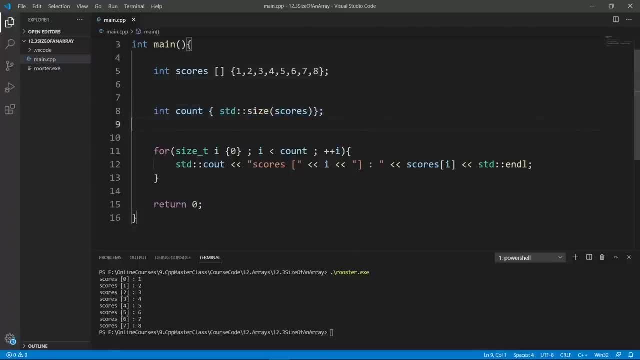 how did we do things before c, Greenspine, C++17.. How did we do things before c plus plus 17.. because std size was introduced in c++ 17, let's say that here. before that, we had to get the size of the entire array and divide that with the size of each element in the array and we could use the. 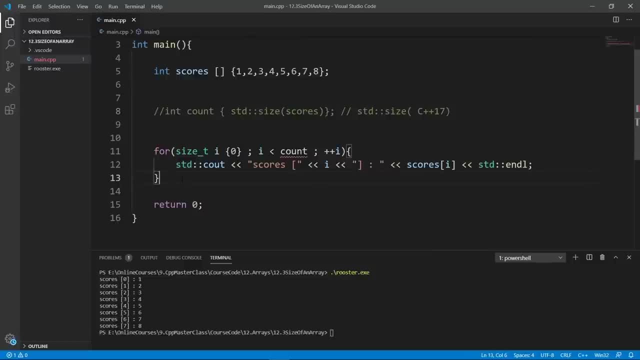 size of operator to do that. so before we do any of that, we want to play with the size of method to really show you what it does. so what we're going to do is say std cl size of scores, the entire array, and we're going to print that and we're going to say std cl size of you know one. 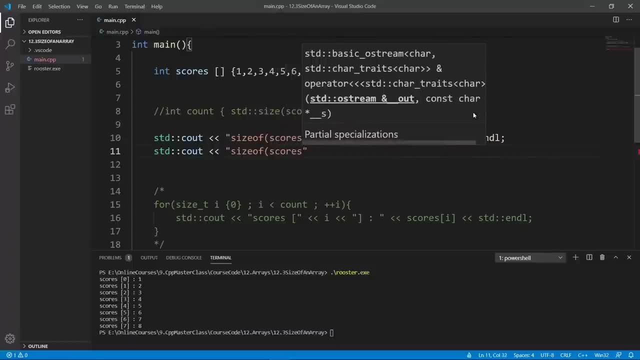 element, let's say scores, and use the first element. this is the easiest thing we can find here, but you can use any element. so we're going to say size of here you, and we're going to say scores, and grab the first element which is at index zero, and we're going to 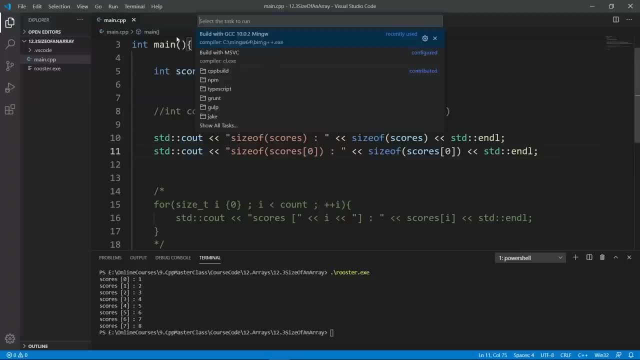 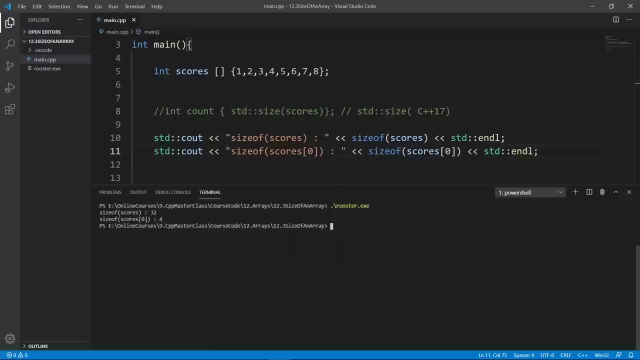 print its size if we build and run this program. we're going to build and run and the build is good. we can clear now and run roaster. you're going to see that we're going to get. size of scores is 32. the entire array, the size of one element, is four, because we are storing in integers and i want you. 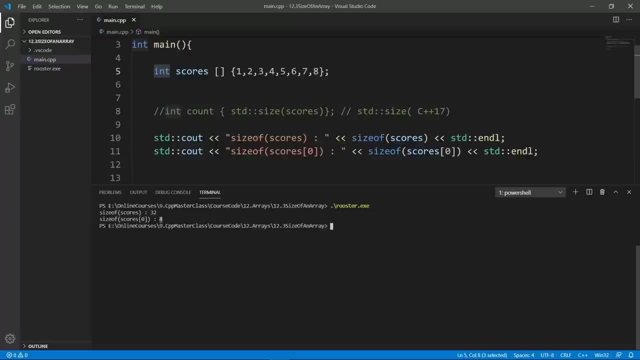 to see that 32 is four times eight because we have in eight elements. so it's going to give you the combined size of all the elements that we have in here if you do size of an array, but if you do size of a single element, you're going to get the size of a single element. so c plus plus developers were clever enough to see. 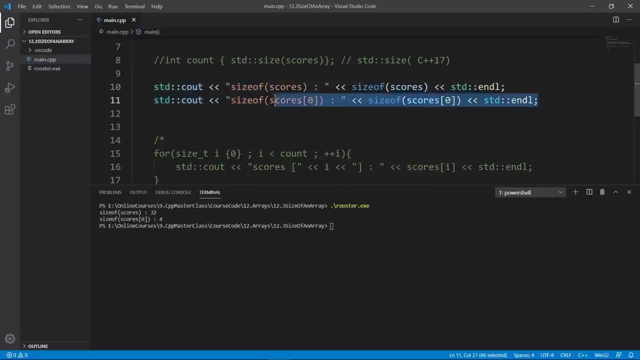 this and see that we could use this information and get the count of elements inside so we can do something like and count, and we're going to assign a value to this in our braced initializer. so we're going to say size of, we're going to say scores, and we're going to divide that with size of and we're going to grab. 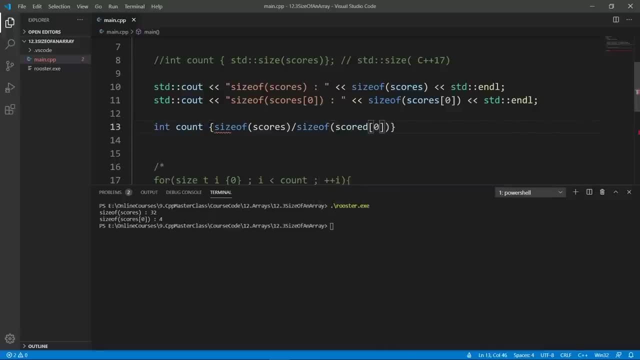 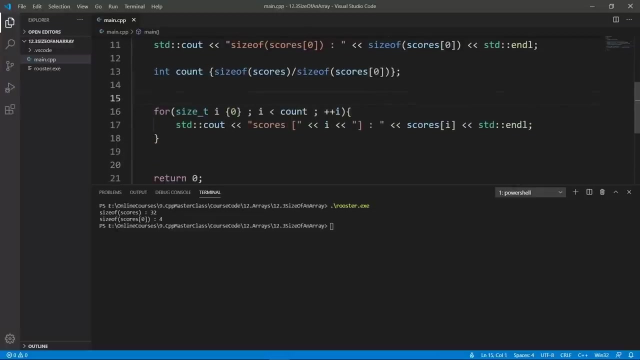 scores. we can really use any element in the array, but we're going to grab the one at index 0 and now we're going to get the count stored in our count variable without using std size and we can uncomment our array here or the code to print the array, and if we run now it is going to work exactly the same thing. 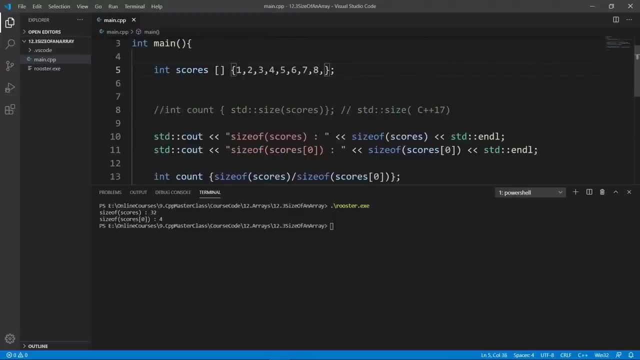 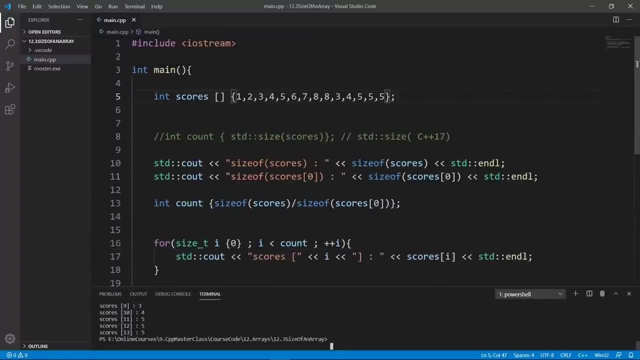 regardless of the amount of elements you have in here. let's put a few numbers randomly and if we build and run, we are going to clear and run rooster and we're going to get all the elements in here and you can really use any of these techniques. just choose what you feel works. 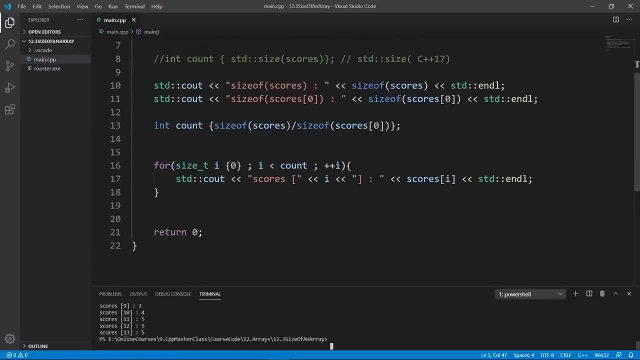 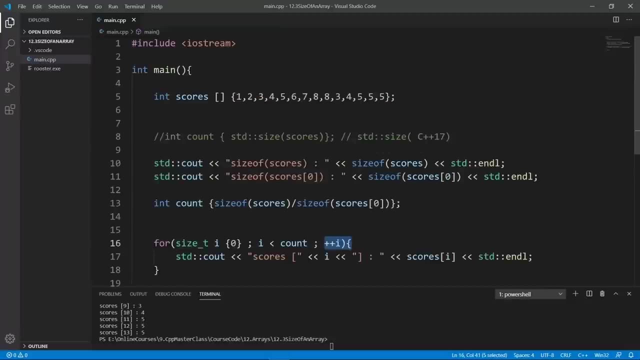 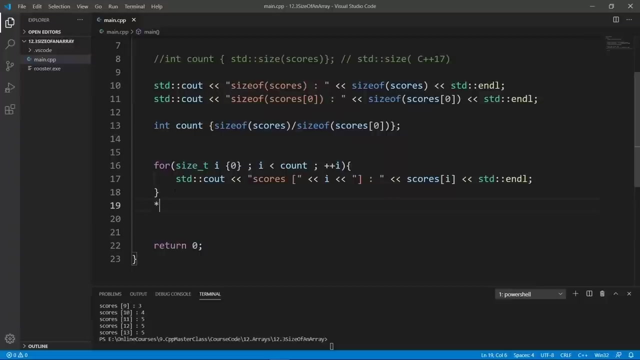 better for you. okay, we are going through all this trouble to set up a neat array, so we're going to do the test. we're going to increment. this is really too much work to try and get data from a collection like an array, so what we can do instead is comment out all this. 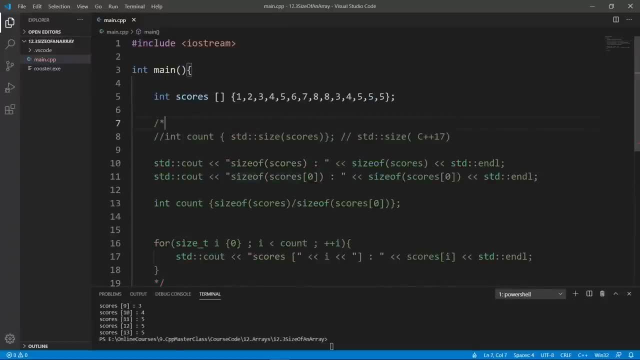 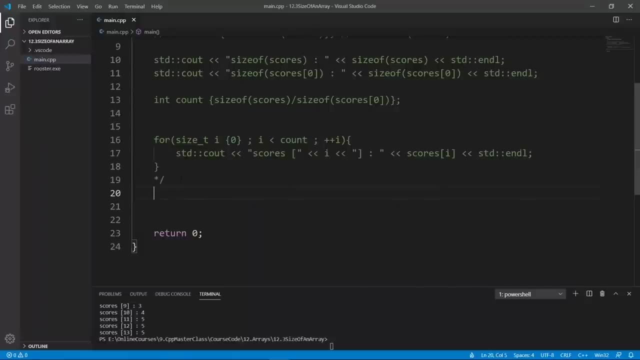 hard work here and we can use the range based for loop, as we have seen before, and it is ridiculously easy and convenient to work with. so what you can do is say: for auto i we're going to do type deduction on whatever it is we have stored in our array. so we're going to put a column and say: 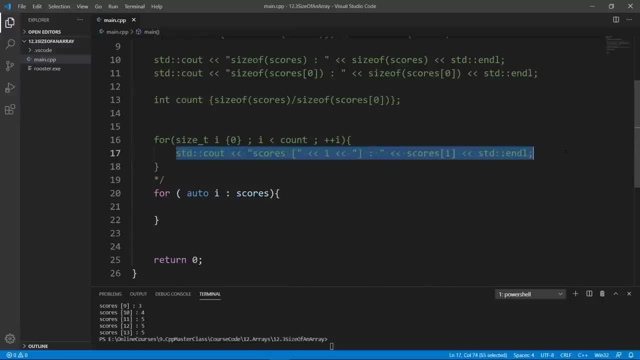 scores and we're going to print out the element. so let's do that. we're going to print stdc out and here we're going to say value, let's say value in the array and we're going to say i, and this is going to print out the all the elements. if we do a right, press d d d off. and then we're going to do this, Воの Simplify Nicknames, andين and these elements. 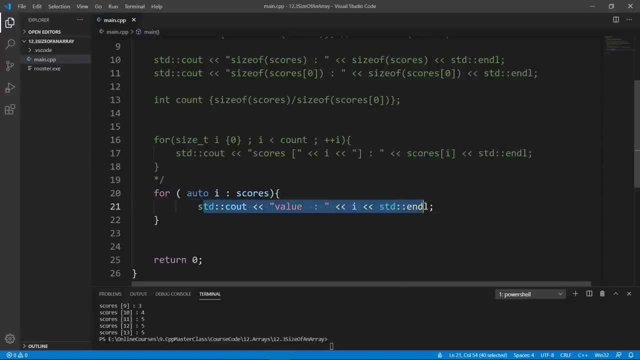 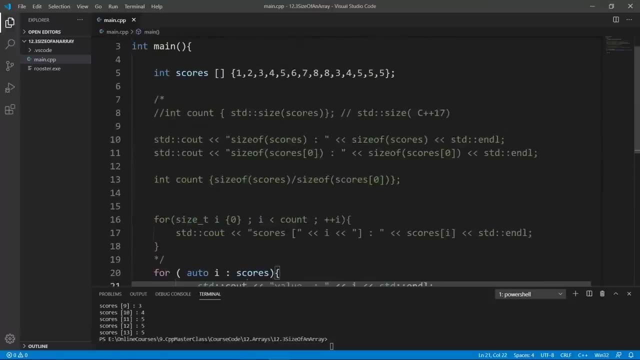 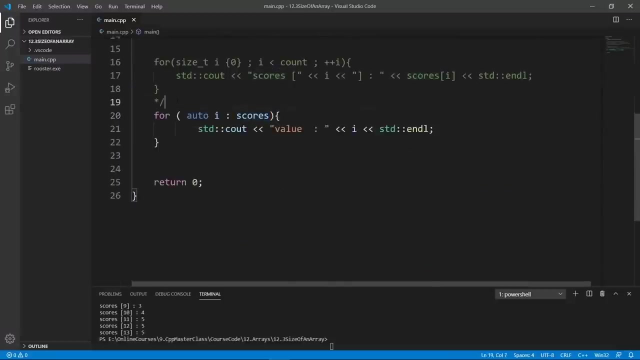 and we can work with the values inside if we want that. but you see that we have lost the information on the indexes. so if you really need the indexes, you will need to go through something like this, and if you just need the values in the array, ranged based for loops are going to be really. 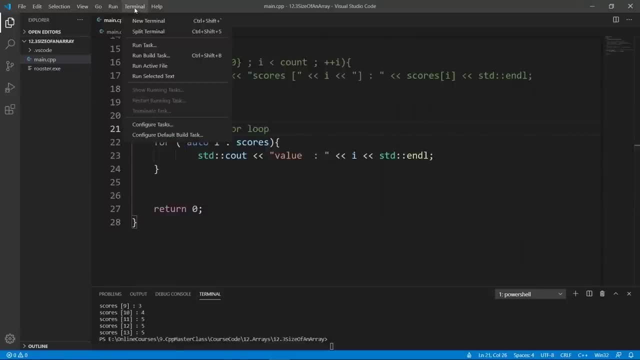 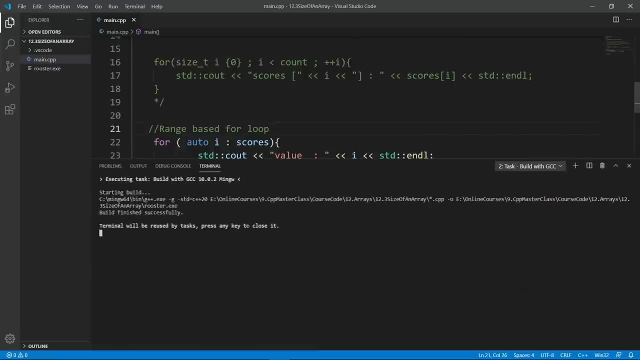 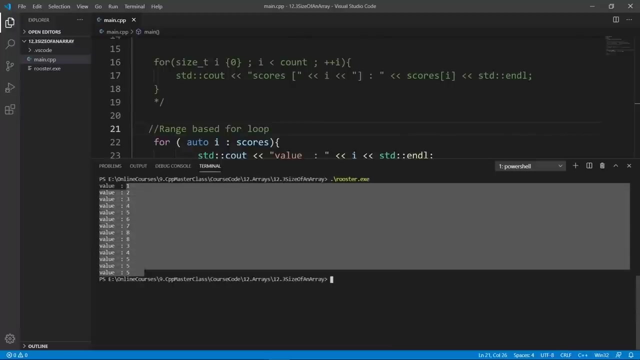 cool. let's say, range based for loop, and if we build and run this, it's going to work pretty well. so the world is going to go through. let's bring this up so that we have some breathing room. we're going to clear and the run rooster and we're going to get our elements printed out here. 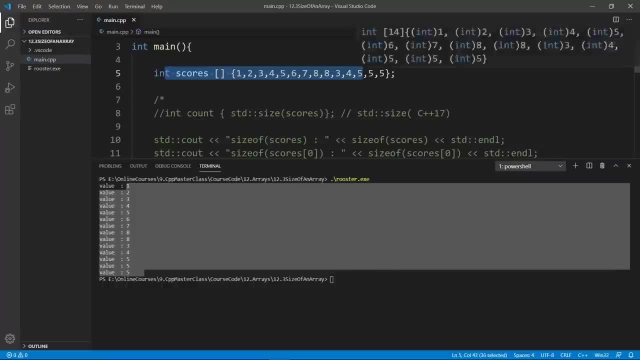 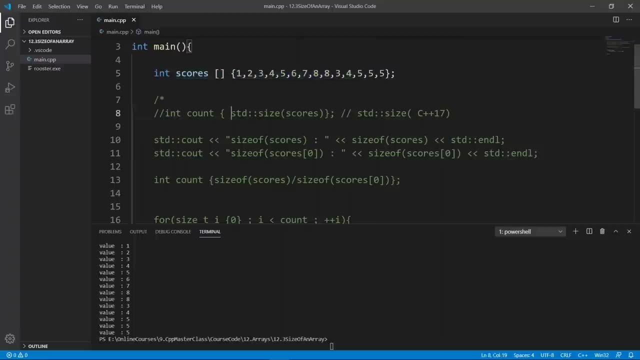 and you see that it is the exact same thing we have in scores here. so this is really all we set out to do in this lecture. i just wanted you to be aware of the std size facility that we have in the c++ standard library if you don't want to use it for. 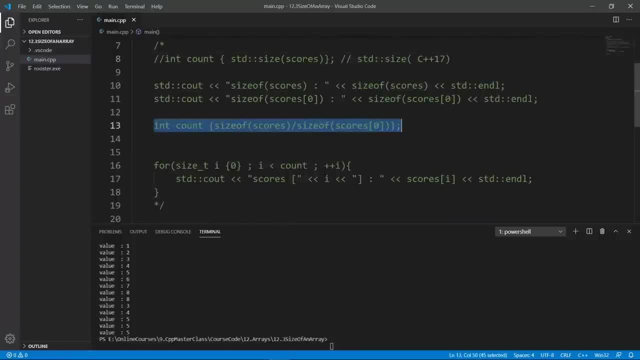 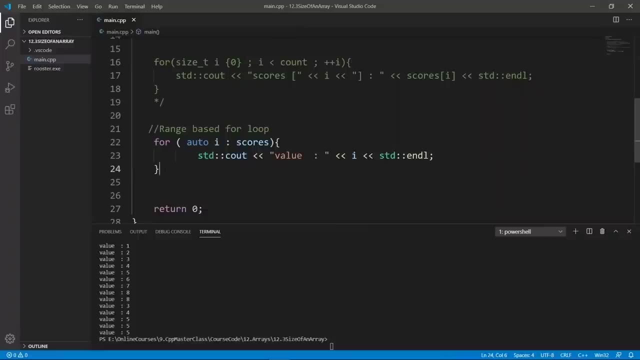 any of your courses. you can use it for any of your courses. you can use it for any of your courses. reason: you can also go in and do the division we did here to get the count of elements in the array and do your best to try and use ranged based for loops because they make it easier and cleaner to. 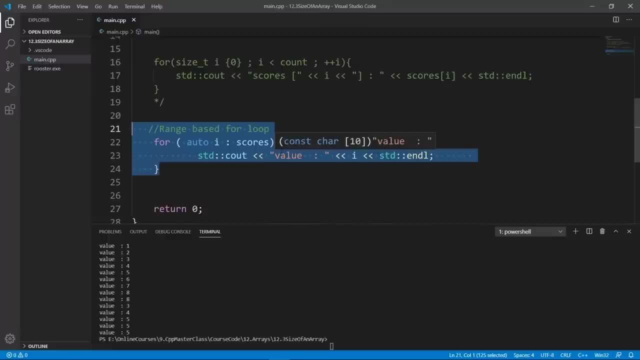 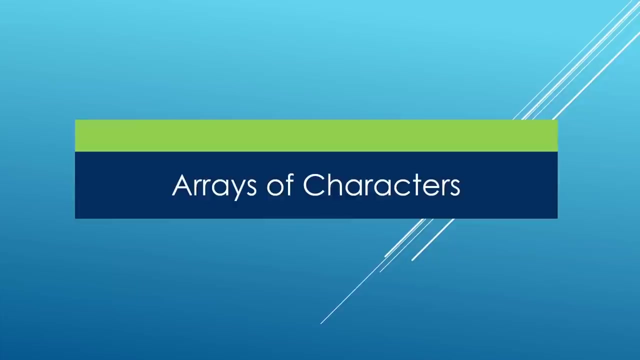 get data from a collection, like we are doing here with an array. we are going to stop here in this lecture. in the next one we're going to see how we can work with arrays of characters. go ahead and finish up here and meet me there. in this lecture we're going to work on array of. 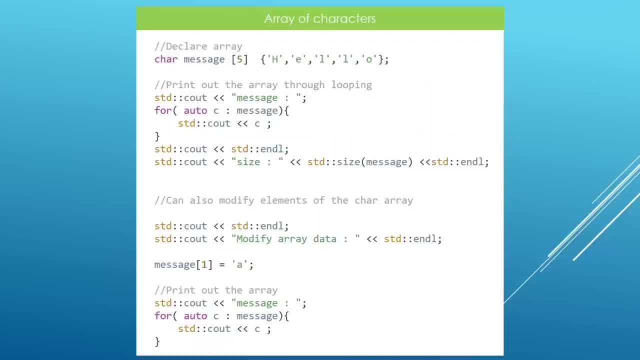 characters and show how special they are. you can declare an array of characters just like any other array. so here we have an array called message. it stores elements of type character, the size is 5 and we initialize it with a bunch of characters. if we want to print it out, we can loop like we loop. 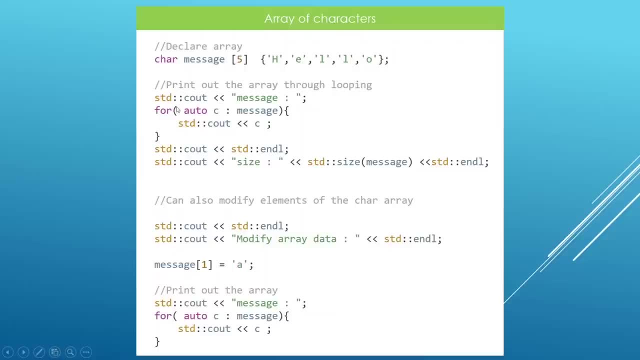 through any other array. in this case we're going to be using a range based for loop. we say for auto c, we pass the message and then we're going to be printing each character in the message and if we do this we're going to see hello printed out on the console. we can also modify elements in. 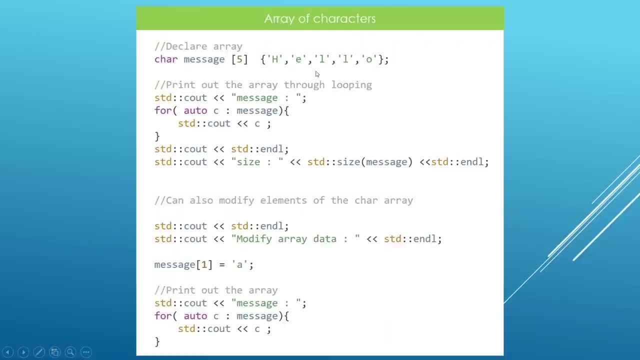 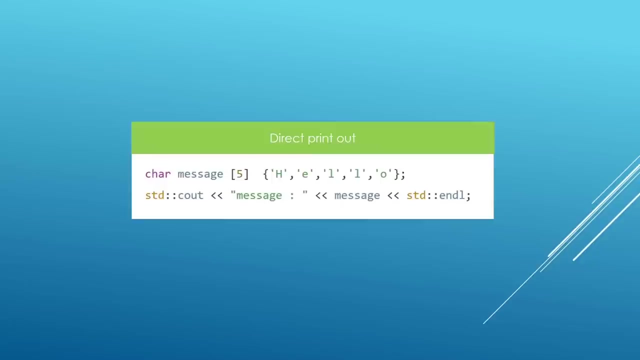 our array. for example, we can say message 1 and change the e here to an a and if we print out, we should see hello printed out on the console. nothing really special so far. the cool thing you raise is that you can print them to the console directly without even doing the loop you can do. 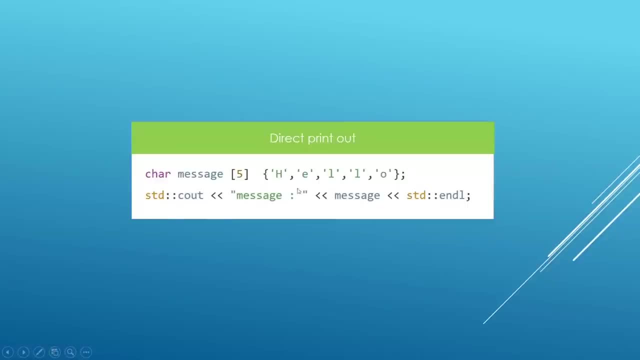 something like this you can do: stdc out, you say whatever you want to do in quotes here and you're going to print the message, but sometimes this one to do what you expect, because only proper c strings can be printed on the console and what makes up a proper? 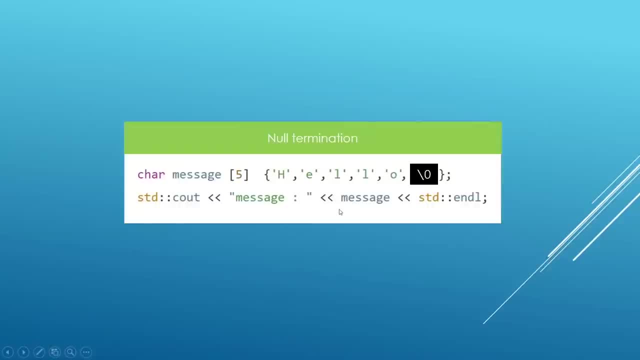 c string. a proper c string has this thing. you see, on the end here, this backslash zero is called a null termination string and it is what is going to tell c plus plus that we have hit the end of the string and we are going to stop printing it. if we are printing with things like 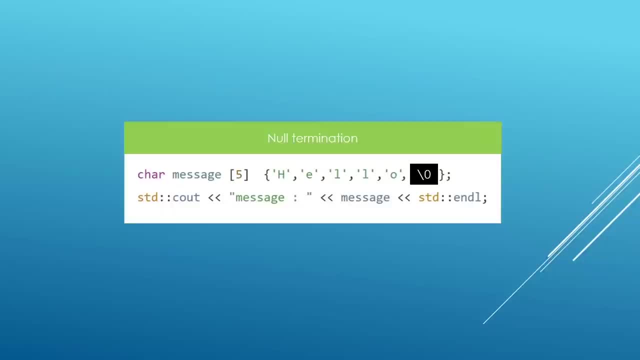 stdc out. so this is really important to be in your strings. if it's not there, it may work, but sometimes it's also going to print some garbage characters after this, because what tells stdc out that we have reached the end of the string is this backslash. 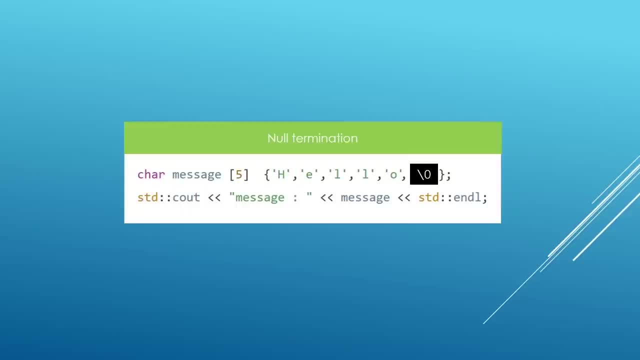 zero here. if it's not there, it's going to keep printing until it sees one, and then you're going to probably have some garbage characters added to your string, and that's not what you want. so to have your strengths printed out correctly, be sure to have n, this null termination character, here, and 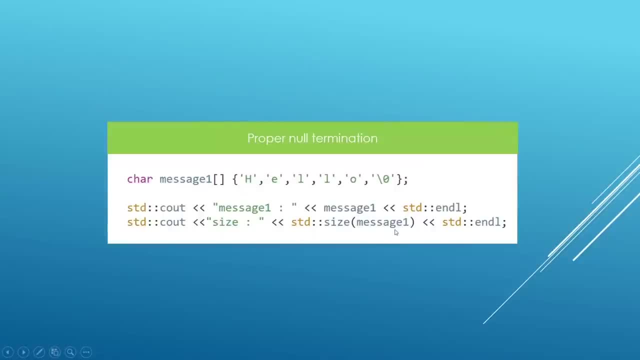 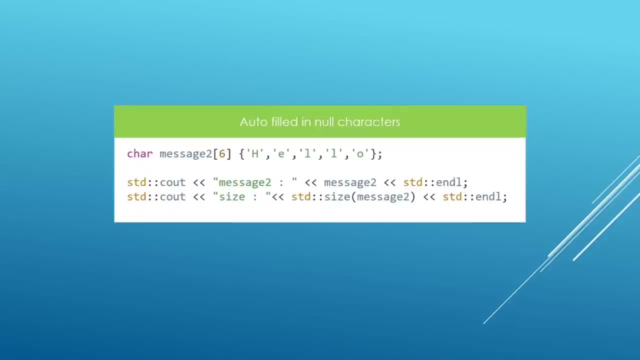 if we print it out, we're going to get it and we're going to see the size printed out properly if we do things like this. but it is possible to get this auto filled for us. if you look here, we have a character array called message2. inside we have said that we need six elements and we say hello. 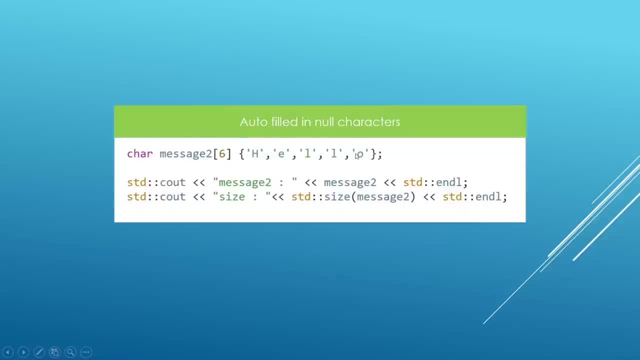 so we have one, two, three, four, five elements, and the elements we don't initialize properly is going to be initialized with a zero version of a character and that happens to be the null terminator of the null termination character. so this is going to print correctly and we're going to have 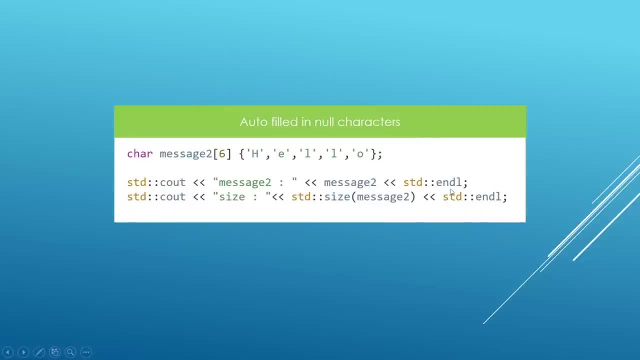 the backslash n appended to this for us by the compiler. but be sure you understand the difference between this and this: here we have specified the size to be a five and we are putting in five elements. so we have no null character appended to this strength. but here we have saved that we can put in six elements and we have only. 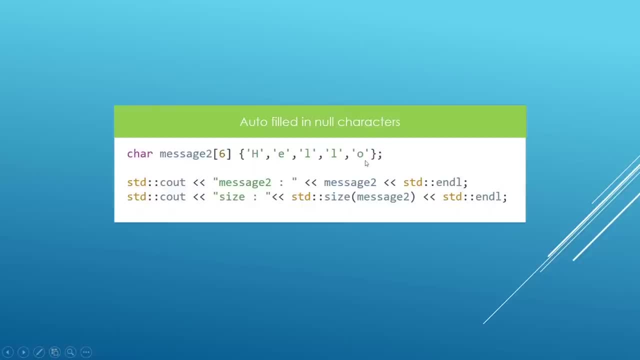 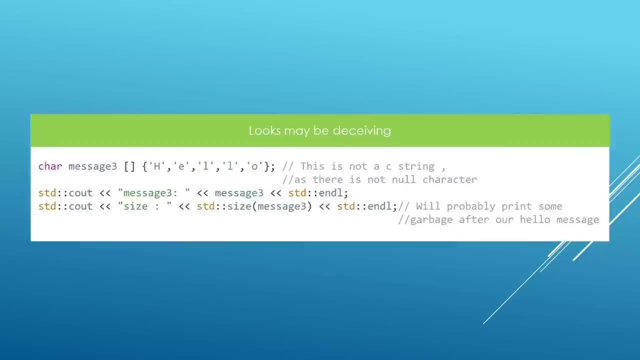 put five and the compiler is going to auto fill in the null terminating character. these two things are different, and make sure you understand the difference, okay, so now take a look at the look at what we have here. we have a string, we didn't specify the size and we just initialize. 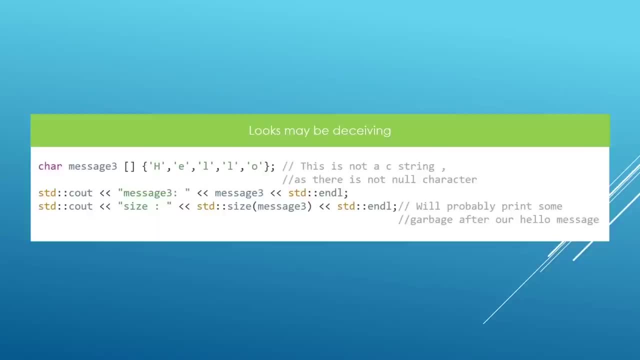 it with hello, someone might think, ah, this is also going to auto fill. but it's not, because the compiler is going to deduce the size of this array using what you initialize it with, and you didn't put in a null character, so it's not going to be accounted for. you're only going to have this here. 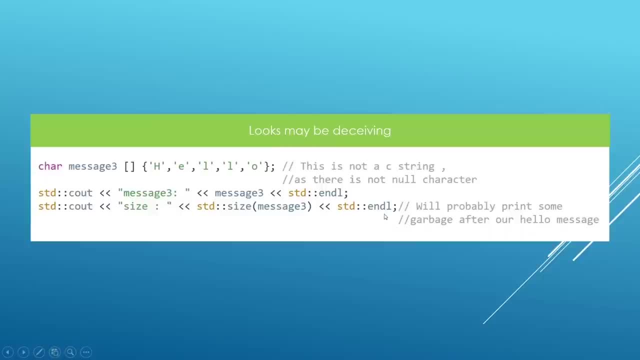 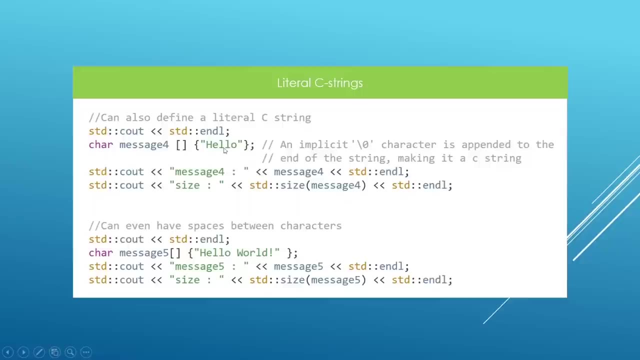 and if you print this out you may get garbage characters appended to your string here, so be careful. but it is possible to do literal c strings and only say hello like this in quotes, and you're going to get the null terminating character appended to your string here. so if 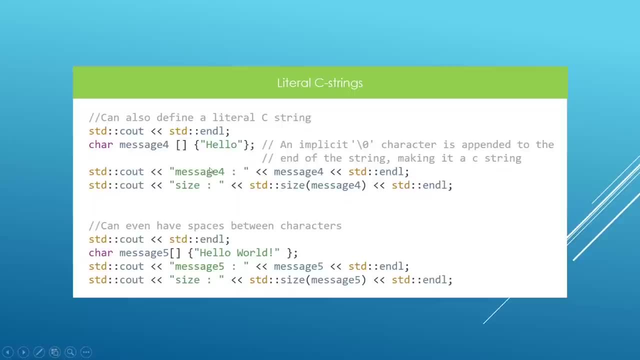 we print this. this is going to print nicely and this is the recommended way to initialize your character arrays. if you want to put in string data like this, you have to use double quotes, and the cool thing about this is that you can even put in spaces between. 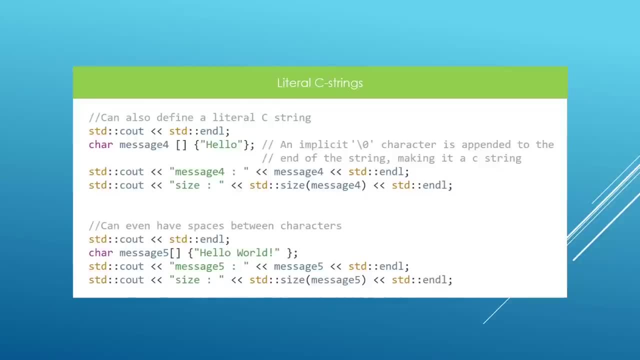 words like this. it is going to work. this really looks like how you would like to type text and store that in your character arrays, and we're going to be using this a lot in the course. again, i want to bring to your attention that character arrays are special in that you can 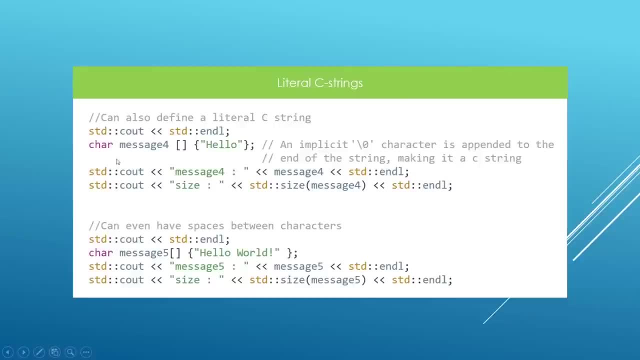 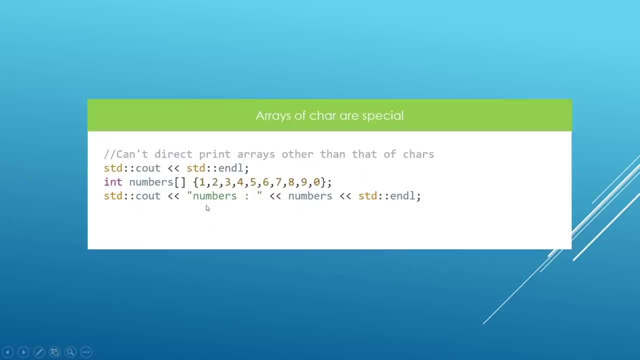 directly print them on the console, like we are doing here. you see, this is a character array and we are saying stdc out message 4.. you can't do this with other arrays, and this is really a lot of work- all i had to share about character arrays. so what we're going to do next is head to. 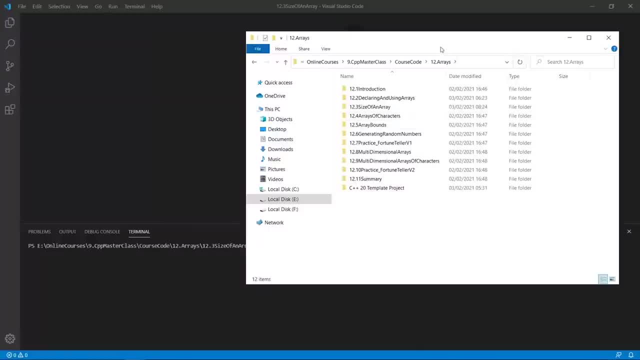 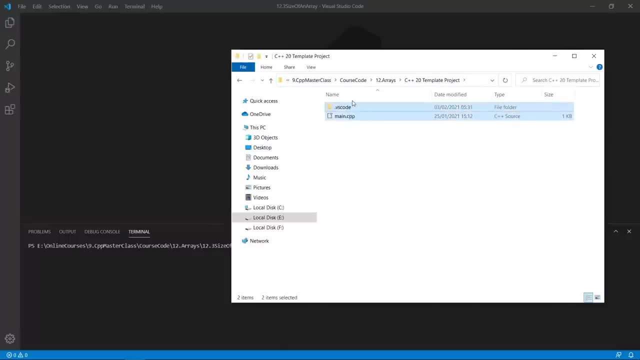 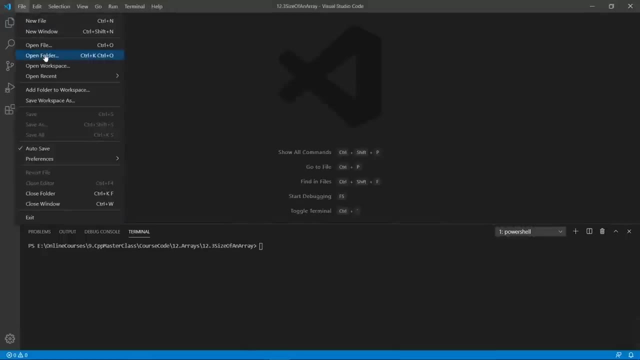 visual studio code and play with us. okay, here we are in our working directory. the current project is arrays of characters. we're going to grab our template project and we're going to copy the files, bring them in here and we are going to open our folder. we're going to open the main cpp file and we're going to get rid of what we don't need here. let's. 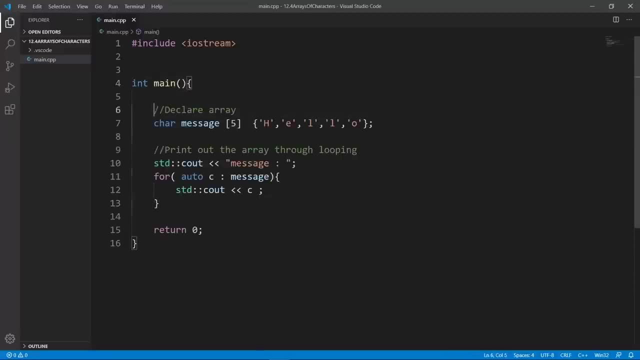 say some startup code, so that we can start playing with this without typing this too much. so we're going to declare an array of characters, it's going to be called message, the size is going to be five and we're going to fill it with characters like this. so if we do this, we might want to print it. 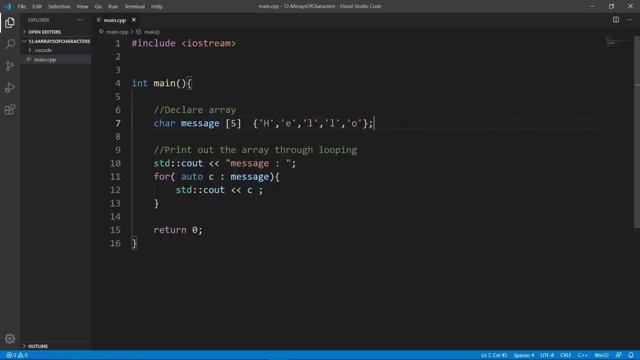 like we print any other array, we're going to use loops and in this case we chose to use a range base for a loop. so we take our toast c, c for character in message and we're going to print out each character. notice that we're going to print out each character. we're going to print out each character. 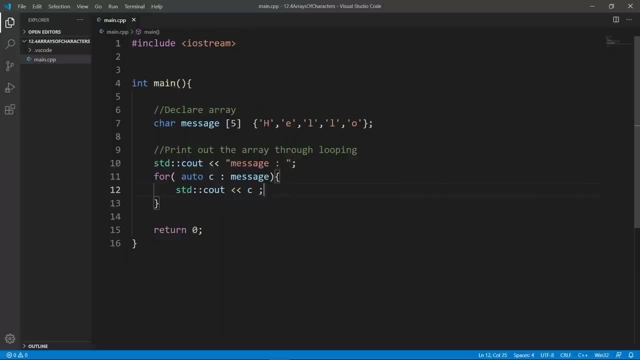 is that we're not adding std endl here, because we want the characters printed close to each other so that we can read this easily, and after this we will need to go to the next line so that the next thing we print doesn't disturb us. so we're going to say stdc out, std endl, and if we do this, we're 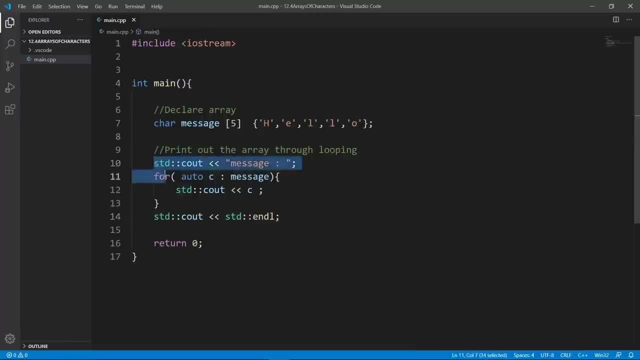 going to see hello printed out on the console, but we had to do too much work to print something simple like hello. but let's do this. we are learning, so we're going to do this. we are learning, so we're going to bring up our terminal and we're going to build with gcc. let's do that. the world is going. 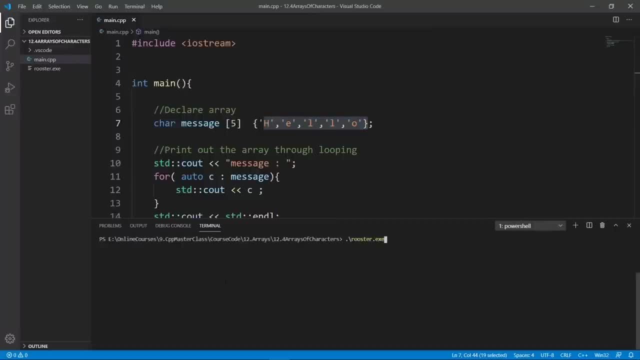 to go through and we're going to clear and run rooster. you're going to see that it's going to say: message is hello and this is what we expect. and this is really how you would declare an array of characters and initialize it with whatever it is you want to initialize it with, but you 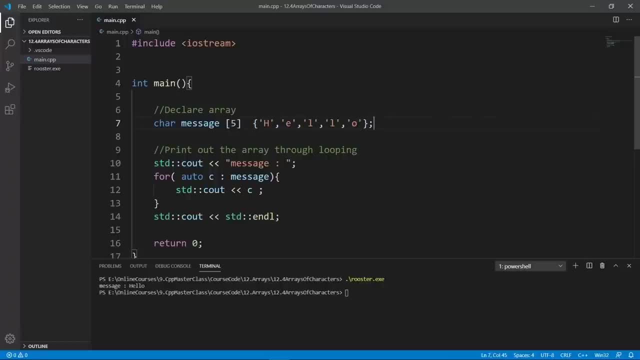 notice that it's really not convenient to put data in here. if you want to store a message, for example, for someone, you don't want to do this thing you see here it's really ugly. it's a convenient and nobody would definitely use your program if you required your users to type things like this. so 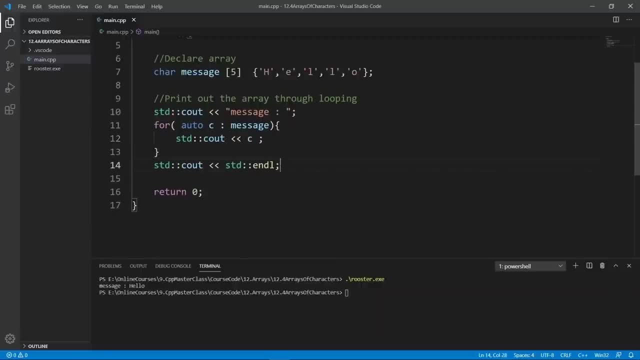 we need to change this and we will. but before we get there, let's also see that we can change characters in our array. so if you look here, this e here is at index 2. so what we can say is say message and we're going to target the element at index 2. 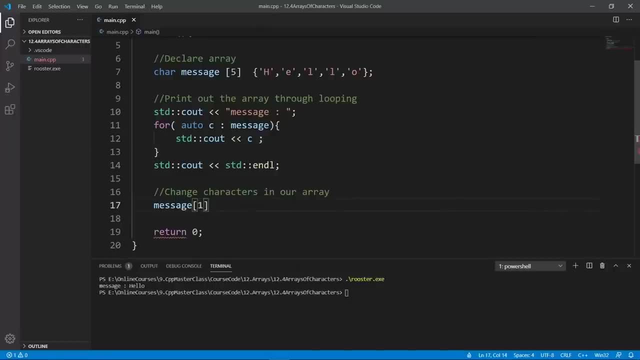 2. oh, it's index 1.. let's use that. so this is index 0, the h and the e is at index 1. let's make sure we get this straight and we're going to store in an a in quotes. remember characters are: 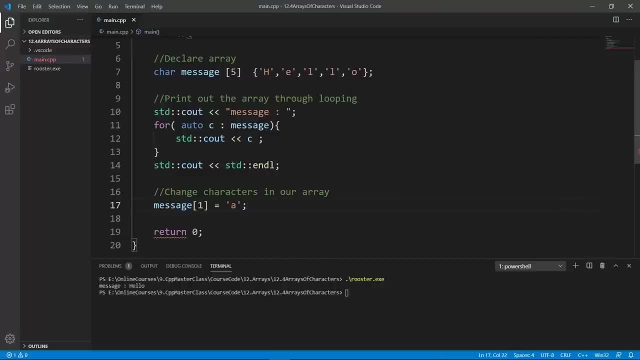 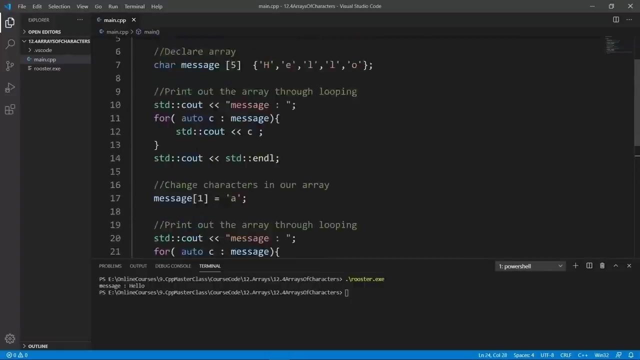 surrounded by single quotes like this. once we do this and we try to print the array out again using our technique here, we're going to copy the code and we're going to paste it down here, just to do this, simply. and if we do this, we're going to see the message printed out here to be hello. 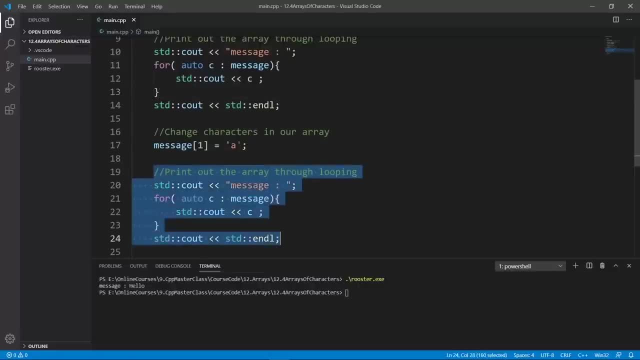 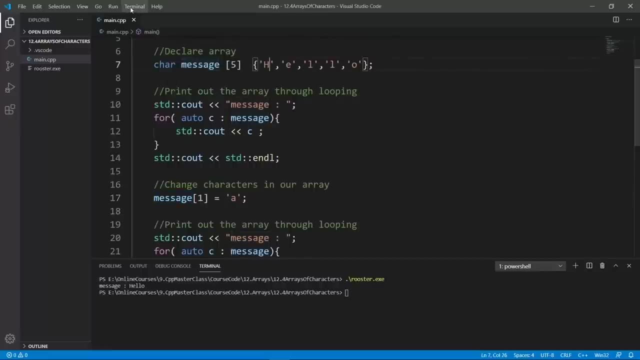 and the second message is going to be: hello with an a, because we changed the second element to an a. it's no longer an e. so that's what we expect. we're going to run the task to build with gcc and we're going to break this up and clear and we're going to run rooster. you see that we have. 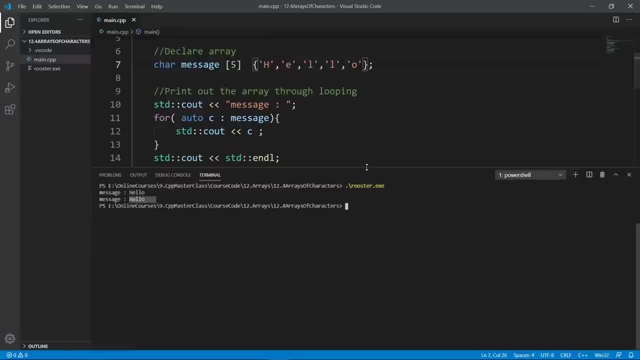 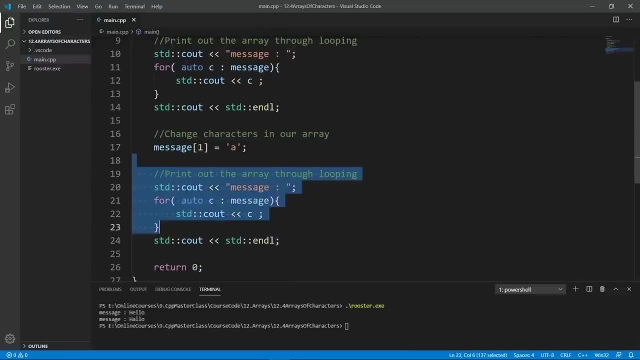 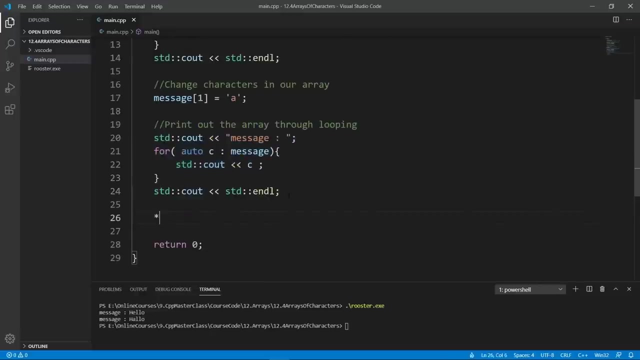 message hello and message hello and we are able to print things successfully. this is really cool, but we are doing too much work really to print something on the console and there should be an easier way to do this, and there is. so what we're going to do is comment this out, because we don't want noise output in the console. 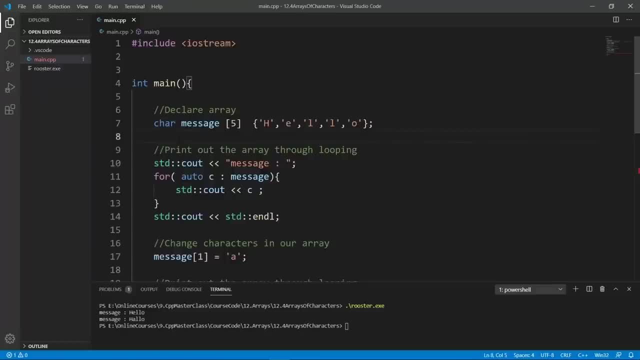 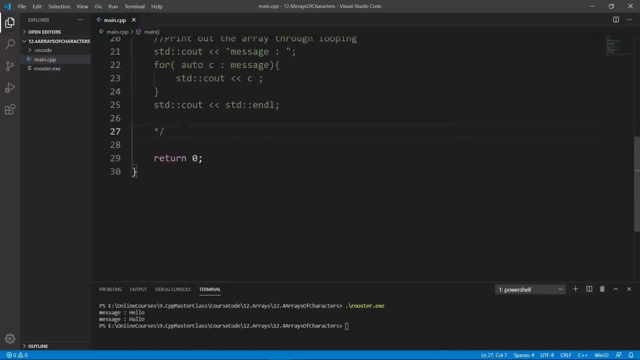 when we try to do something else. so what we're going to do is comment out all we've done so far. we're going to leave in our message here and we're going to try and print it directly on the console so we can say sd, dcl and say message, and we're going to print out the message. 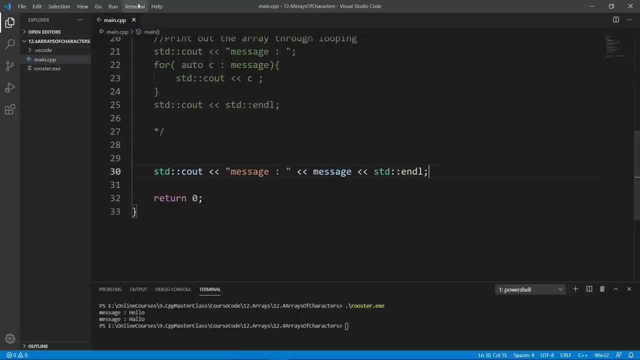 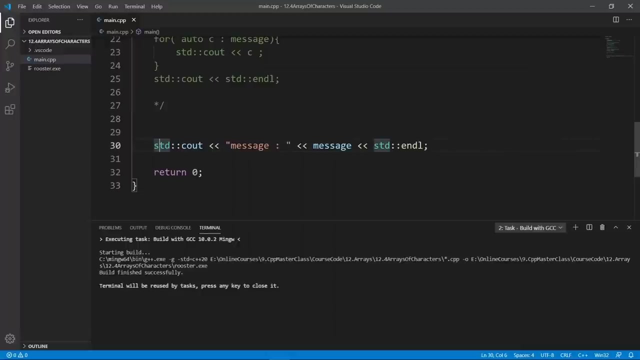 and take a moment and look at this and try to compile this. it is going to go through. it is going to compile because c plus plus supports printing character arrays like this, but, uh, in most times this is not going to do what you expect. let's try and run this and see what we get. 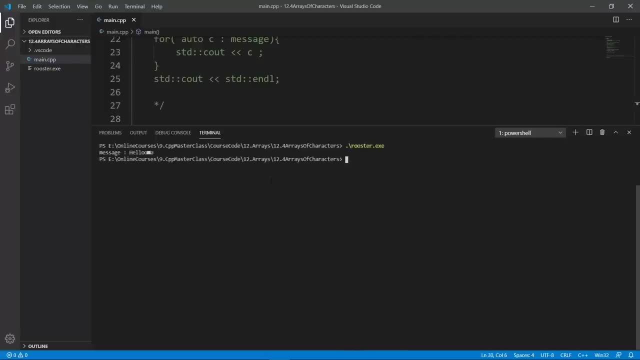 we're going to run rooster and you see that we're lucky to get something that really isn't what we expect. it's printing hello, and you see that we have a bunch of other things, and the reason is what we have discussed in these slides- for character arrays like this to be printed out. 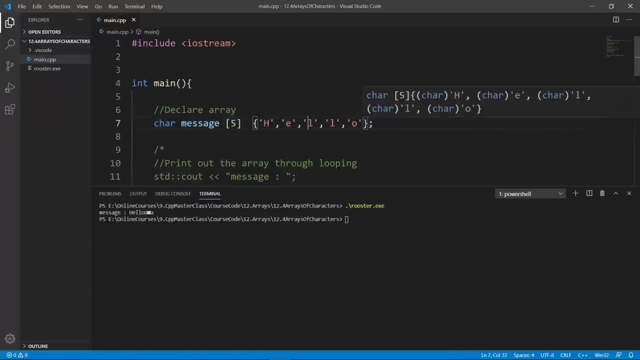 properly on the console. they need to be null terminated. in other words, they need to have the null character, which is a backslash zero. so they need to be null terminated. in other words, they need to have the null character, which is a backslash zero, appended to the string for sd dc out to know that it has reached the end of the string. 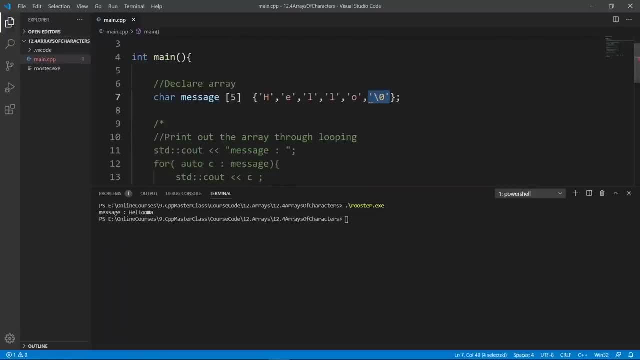 so this is what makes your character strings legal. now you see that we are getting a compiler error because we have overflown the size of the array. i think that's the message: too many initializer values, and this is exactly what we have done. now we can try and change this guy to a six, to. 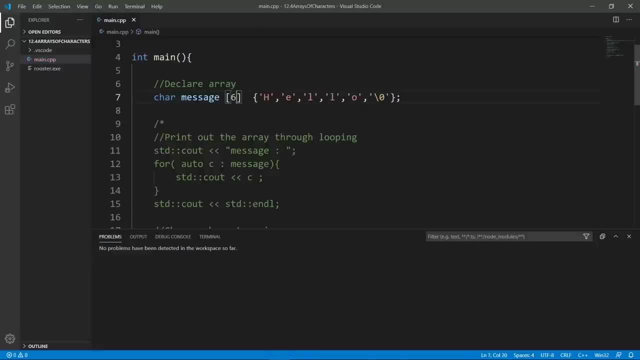 say that we have six elements in here. this wiggly line should go away and if we try to build and run, we're going to build with gcc- let's bring this up a little bit- and we're going to clear and run rooster now. and you see that now we have hello printed out. 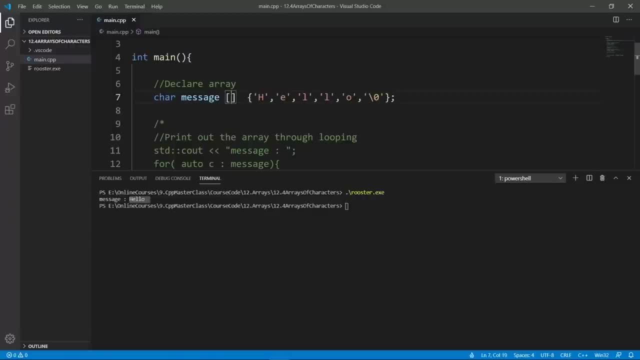 correctly. if we turn this back to five elements and take out the null terminator, we're going to try and build again and we're going to clear and run rooster. you're going to see that we get the garbage back. so for your strings to be printed out correctly, they need to be now terminated. that's why it is. 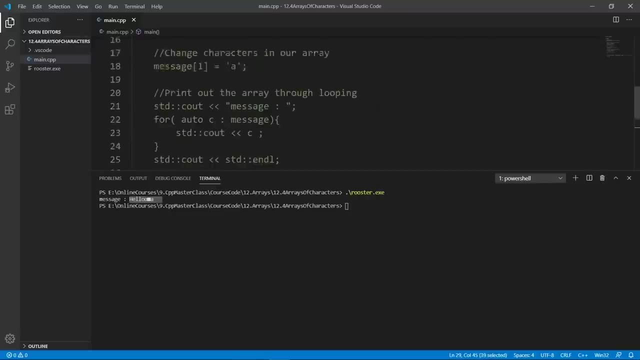 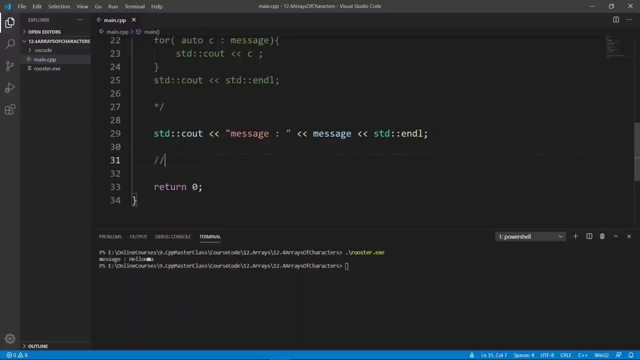 not safe to print something like this when your character array is not null terminated. i really want you to understand this. so in c plus plus, we have a proper name for these strings that are null terminated. a null terminated string is called the c string, because these things come from the c. 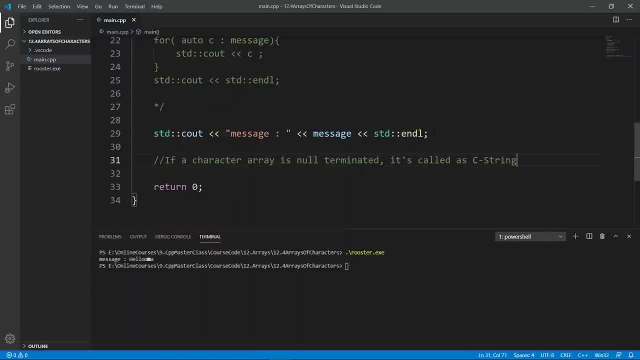 programming language, okay, and we're going to see a little bit more about the c programming language. we're going to see a little bit more about the c programming language, okay, and we're going to see a few ways we can set up c strings now, and the first one is to say car. we can call this message. 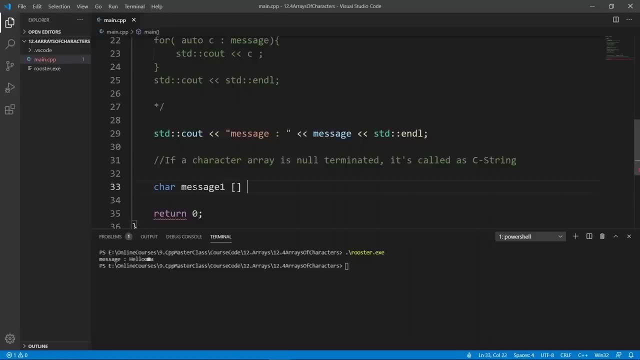 one, and it's going to be an array of characters and we're going to initialize this with hello. let's copy this because i don't want to type all these things here. so let's copy this and initialize this properly. notice that we didn't specify the size, so the compiler is. 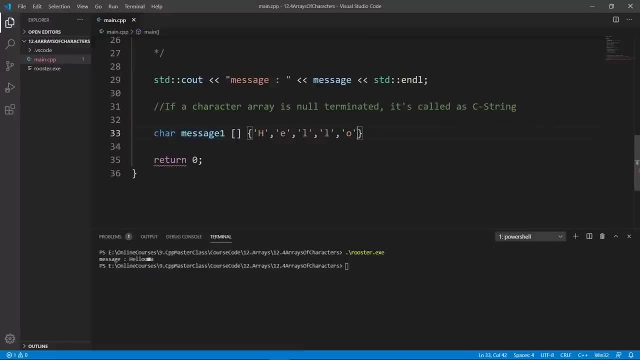 going to get the size from however many elements we put in here and we're going to put in our null terminator here and if we print this, this is going to work and we are going to comment this out and we're going to say that this will give you garbage. okay, if we come down here, we're going to. 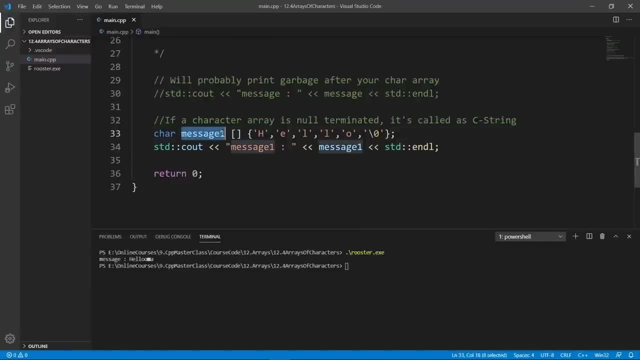 see that we have a car array- it is called message one and we have initialized it with data. we have hello and we have a null terminator here and the compiler is going to deduce the size. so this is going to be a proper c string and we will print it correctly. let's try and see if we can print it. 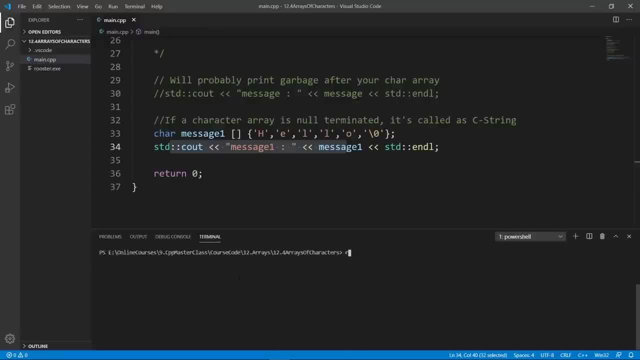 correctly and do this and weld this, the board is going to go through. if we clear and run rooster, we're going to get our message here and this is one way we can set up a proper c strand. the second way is to actually not put in the null terminator but let the compiler 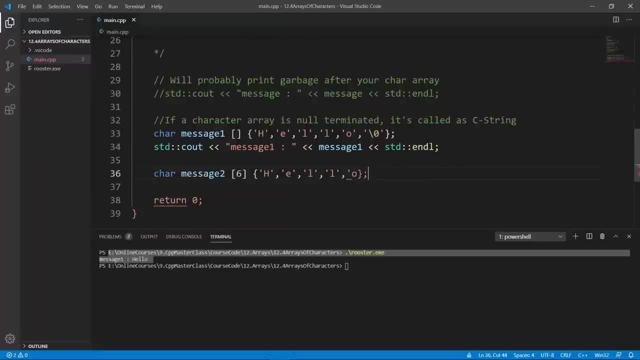 add that in for you and the way we can do that. we can say car message to how we end things here. we're going to put in our code and end this with a semicolon. now what is going to happen is the compiler is going to see that this array is of size six, but we are putting 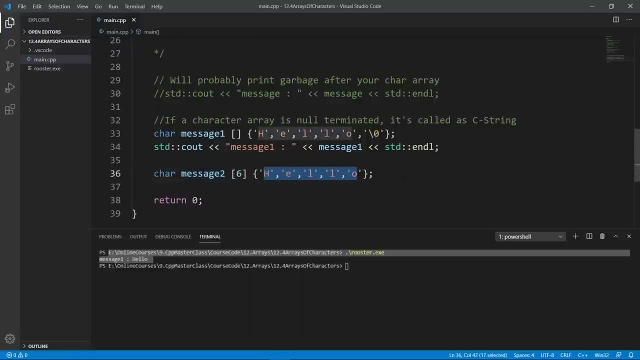 in five elements. so the remaining slots are going to be auto filled and it is going to be using null terminators to auto fill this. then if we try to print the size here, we're going to get a six because the null terminator is added in by the compiler. let's try and print the sizes here. 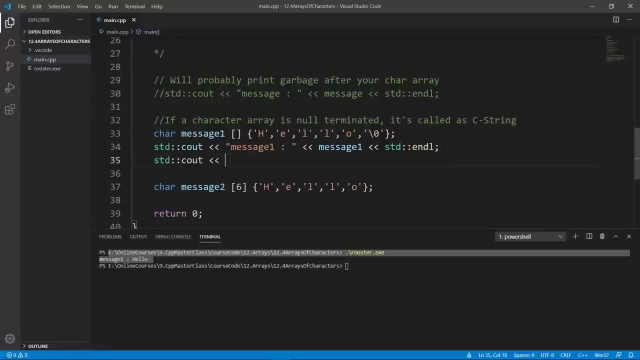 actually, so that you can see these things. so we're going to say size and we're going to say that size of message one, and we're going to put in a new line character, and this should be what we expect. so what we're going to do, we're going to copy this and put that down here, because we're going. 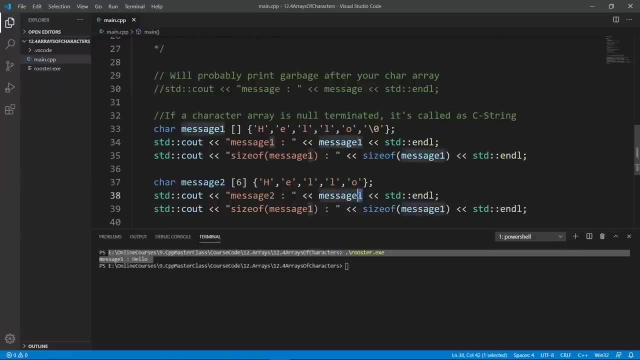 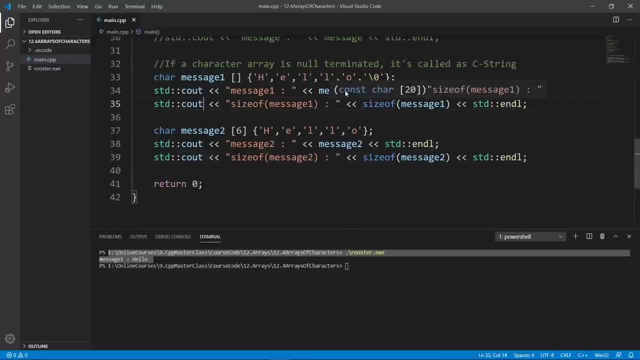 to be doing the same thing for message two. so we're going to say message two, let's select that, this and say size of message two and do size of message two. so what we're going to see is message one and message two printing out, and we expect to see a size of six because both of these 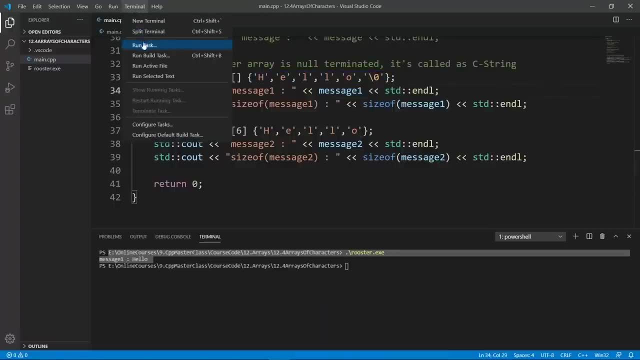 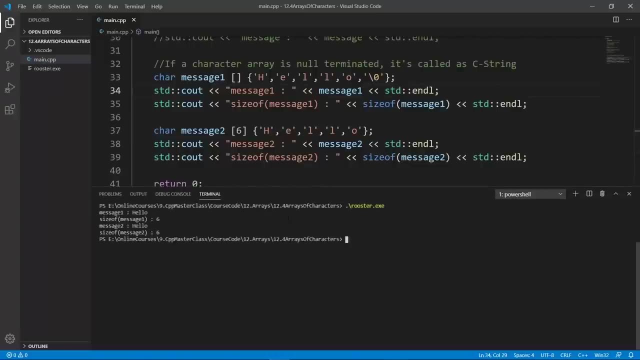 guys have six elements inside, so we're going to run the task to build with gcc and bring this up: clear rooster, and this is exactly what we expect. message one is hello, the size is six. message two is hello and the size is six. and these are a few ways you can declare your character arrays and 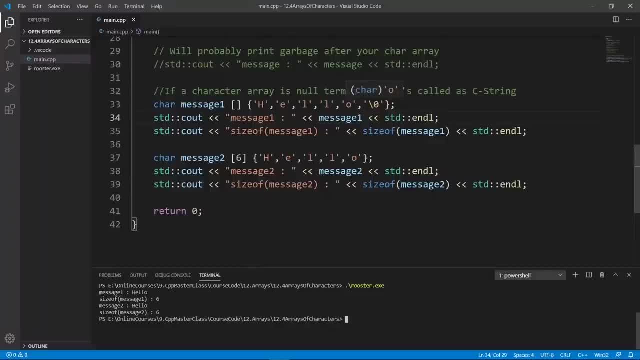 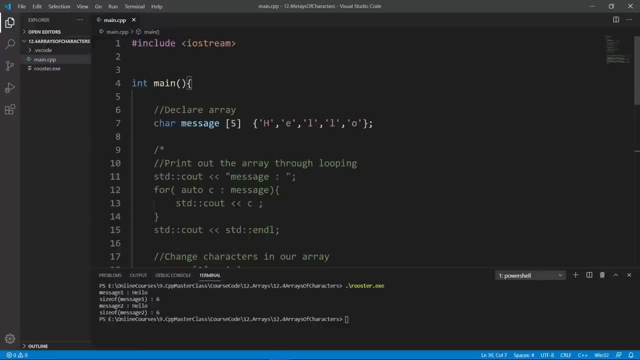 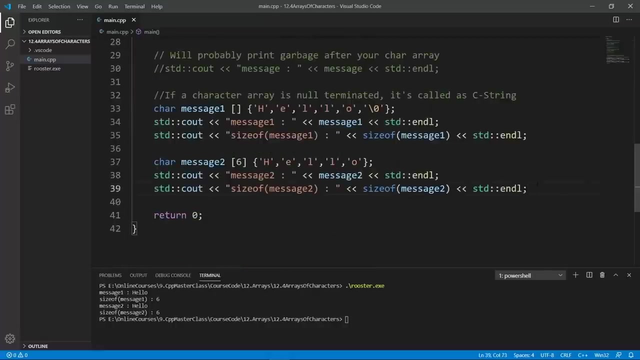 initialize them with proper data. that is going to print correctly with stdc out. make sure you don't do something like we did here by printing message here because it is not null terminated. this is going to give you a lot of problems again. i want to make it really clear that message three here. 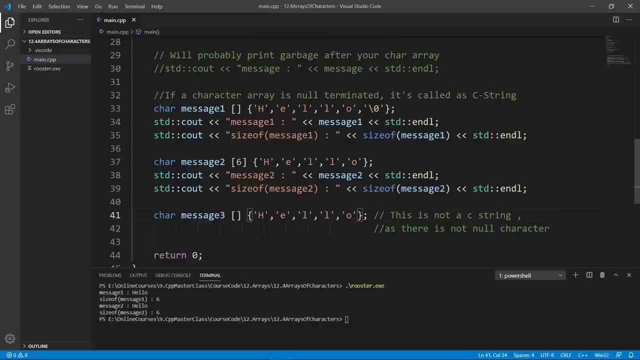 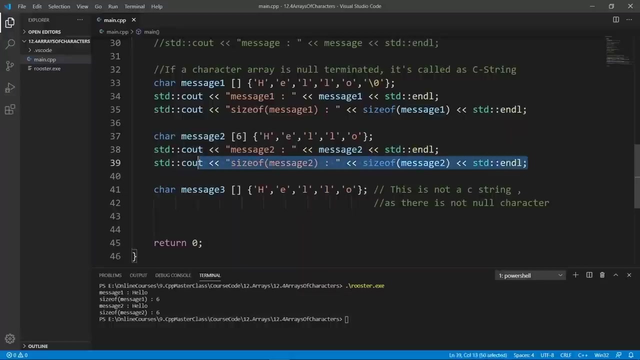 is not a proper c string, because the compiler is going to deduce however many elements we have in here and this thing is going to be of size five and we're not going to have a null terminator and if we print it out we're going to get some garbage. so let's try and copy this so that 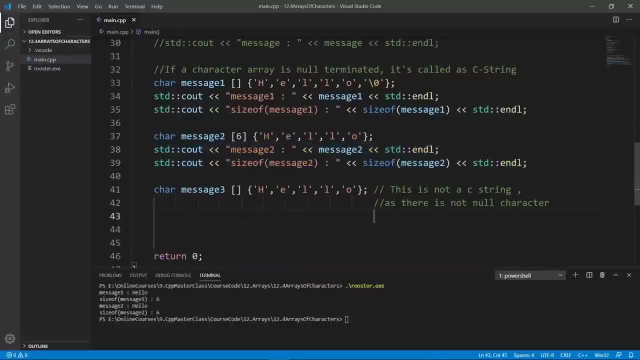 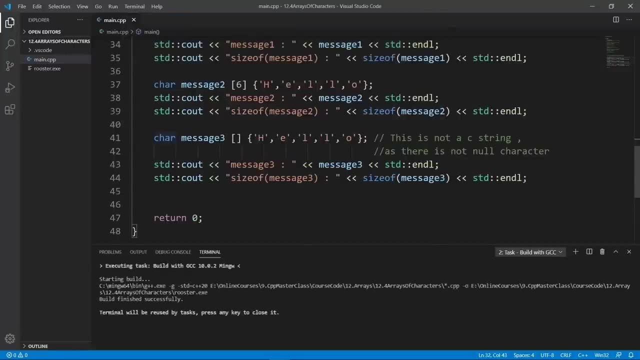 we are consistent with what we've done above here and if we compile with gcc, we are going to compile successfully. but we may get weird things if we print out message three like we do, and you're going to see that the size is five, because we only have five elements in here. so 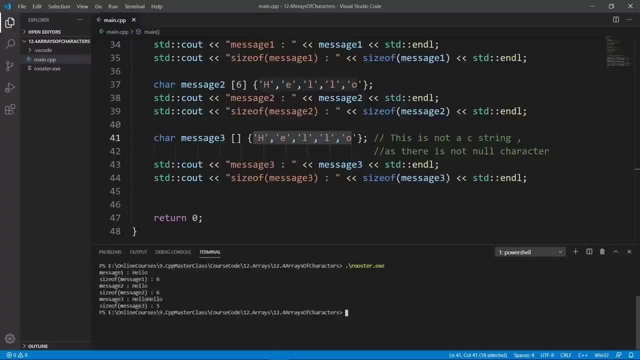 let's clear and run rooster and you're going to see that we have hello for message one, we have hello for message two, but for message three we have things we don't expect because it's going to keep printing and it's going to go over bound and it's going to stop when it hits the first. 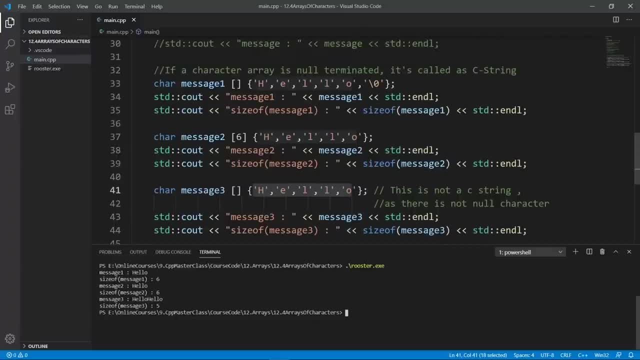 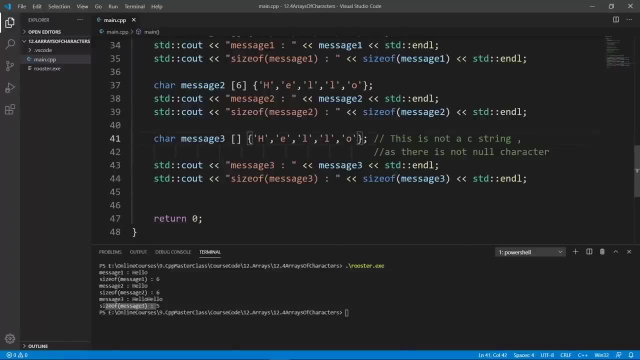 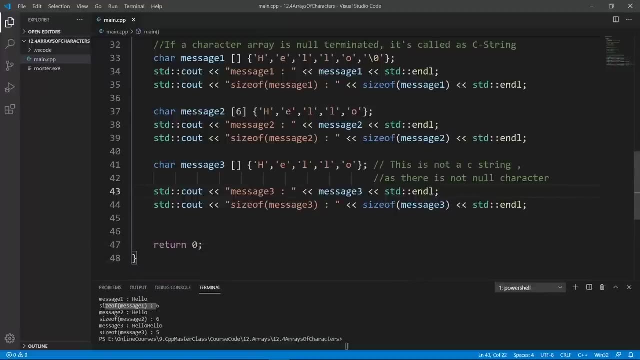 null terminating character like what we have in here. okay, so this is not safe. don't do it. make sure your strengths are null terminated if you intend to print them with sddc out like this, okay. so working with character arrays like this to print messages and do all kinds of crazy things is nice, but it really isn't convenient, as i said before. 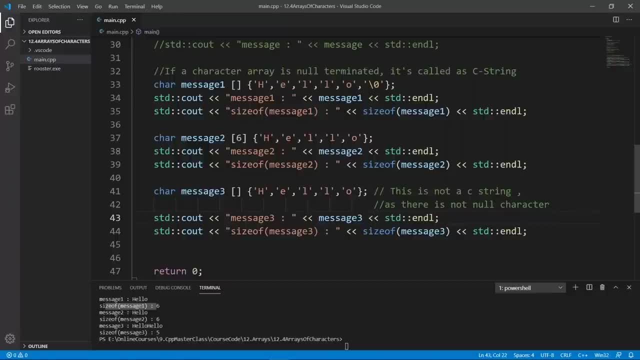 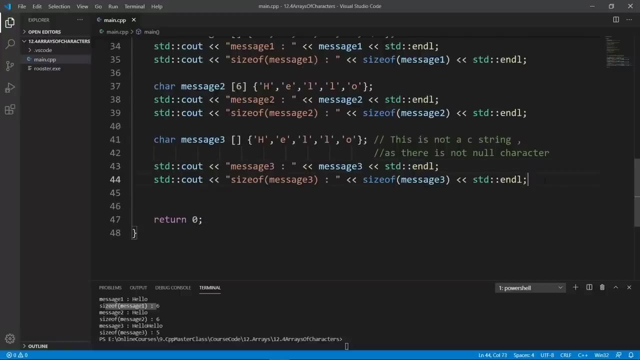 you wouldn't expect your users to type characters like this by surrounding them with single quotes. this is really ugly and it is painful to do if you want to do some productive work. so c++ allows you to use what we call string literals and we're going to see an example of that down below. we're going to say string literals and what we can do. 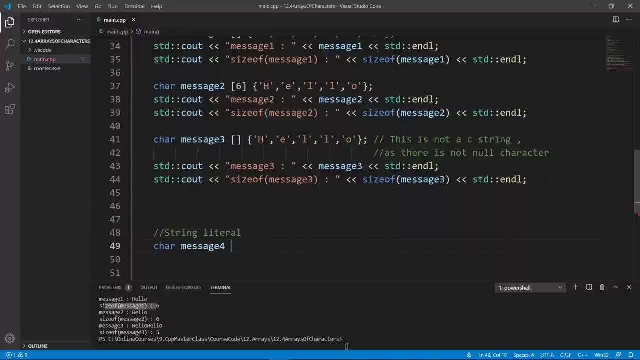 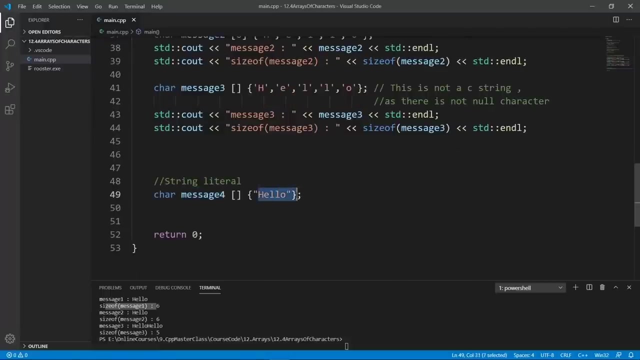 is car message form. it's going to be an array, as usual, and we can initialize it with a string that is surrounded by double quotes, and what this is going to tell c plus plus is, you know, take this things, bracket it into characters and store this in this array here and make sure you properly. 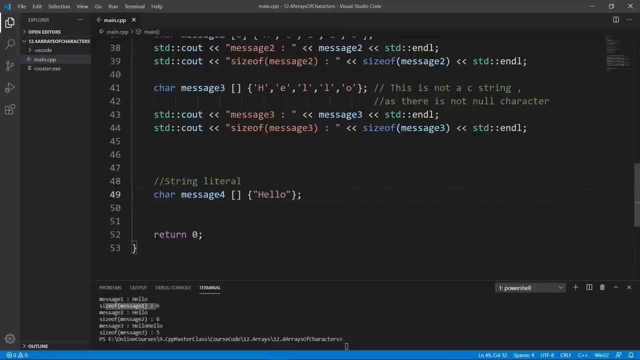 null. terminate this string here. so if we print the size of message four, we're not going to get five, we're going to get six, because c plus plus is going to see these double quotes and know that we intend for these things to be properly now terminated and it's going to. 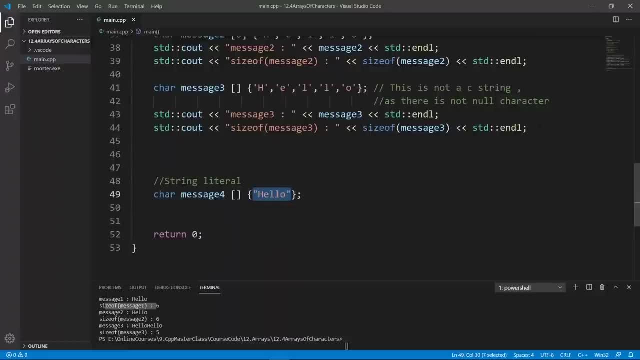 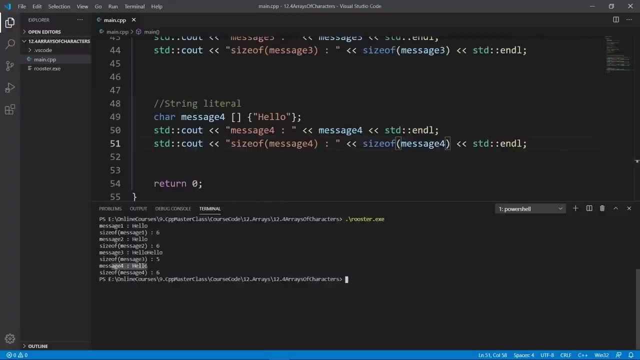 add a null terminator. so let's try and print this out so that we really don't want to have a null terminator. so let's try and print this out so that we really are sure- and we're going to weld this with gcc as we always do- the world is going to go through. let's go up and clear and 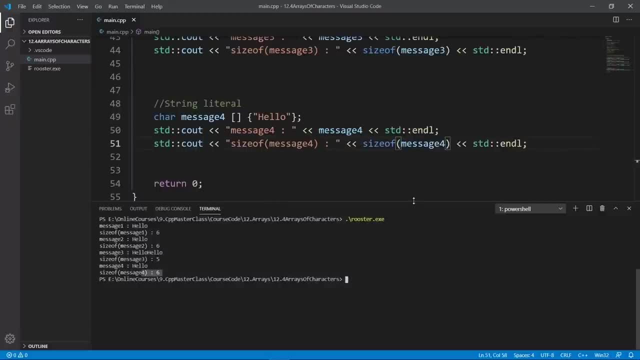 we're going to run rooster and you see that message 4 is hello and the size is, indeed is 6.. so this is one way we have to do things, and we can even put spaces and do all kinds of crazy things, and it's really cool and if we try to weld this, we're going to get the proper message printed out. 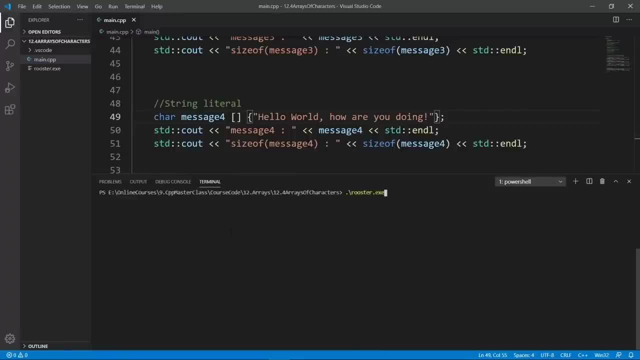 the world is good. if we clear and run rooster, we're going to see hello world. how are you doing? and this is really cool. so from now on, if we need to store a string in our program, this is how we're going to do it, because this is much more civilized and it is how you would really like to type. 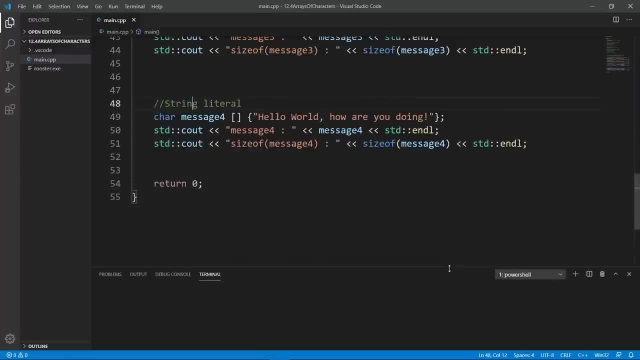 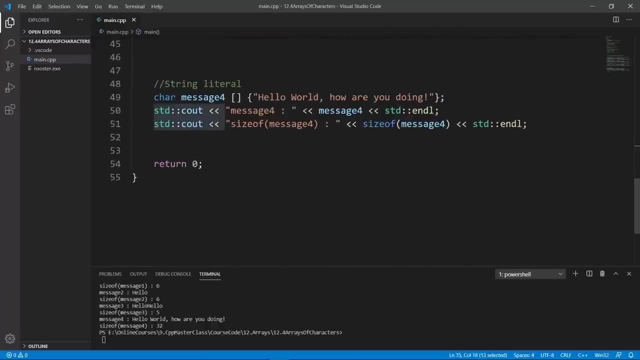 characters in your program. i have said that character arrays are really special because you can directly print them out with stdc, out like this: i want to prove this. so we're going to try and declare another array, so we're going to call this numbers and we're going to make this an array and we're going to initialize with one, two, three, four. 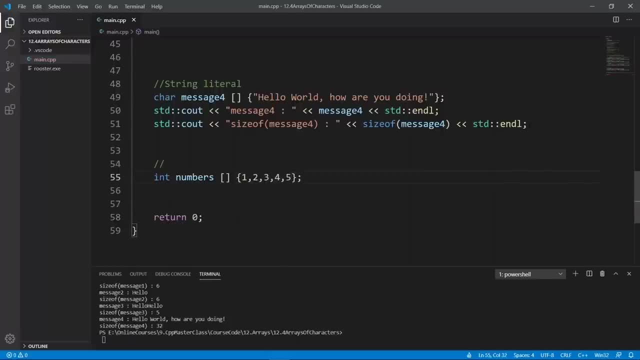 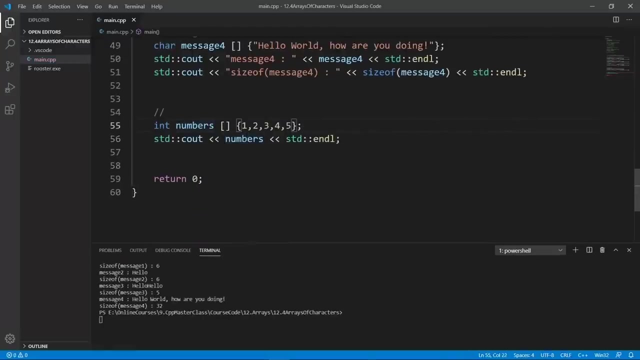 five. this is going to do and we're going to put our closing semicolon and we're going to try and print this out. we're going to say std c out and say numbers, let's see what we get. let's try and compile this and see what we get. it is not actually going to give us a number, but it is going to give. 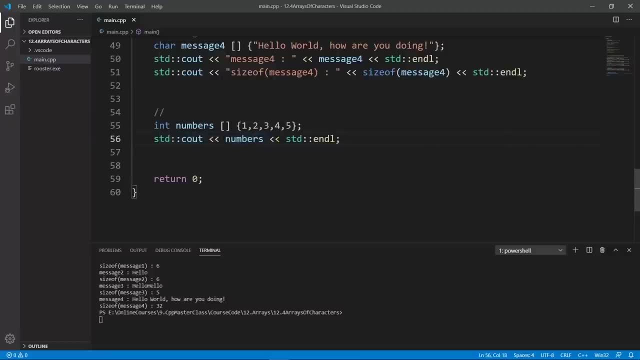 us a compiler error, but it's not going to print what we expect and let's put a message here so that we know that it is this thing we are seeing here. so we're going to say numbers and we're going to put a column here and we're going to build this with gcc and we're going to clear and if 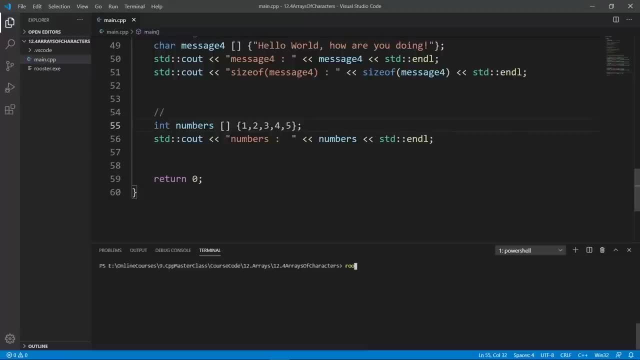 we run rooster, look out for the output that says numbers here. so let's run rooster. it's not a one, two, three, four, five. it's something we don't really know, and we will get to understand what is happening here in the next chapter. for now, know that you can't directly print arrays other than those of 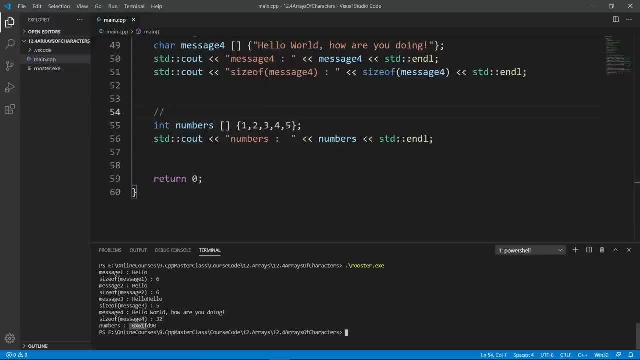 characters. if you try to do that, you're going to get weird numbers printed out and we're going to understand why this is in the next chapter, so let's say that here. okay, this is really all we set out to do in this lecture. i hope you found it interesting. character arrays have a few things. 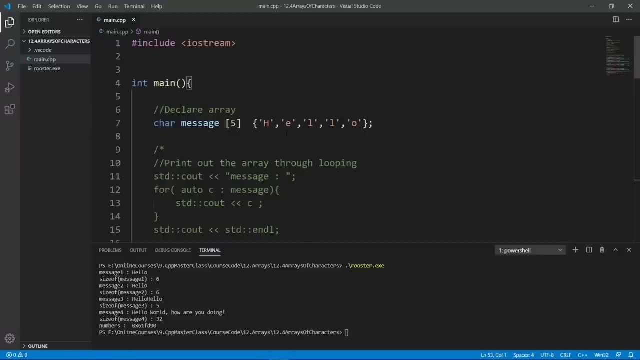 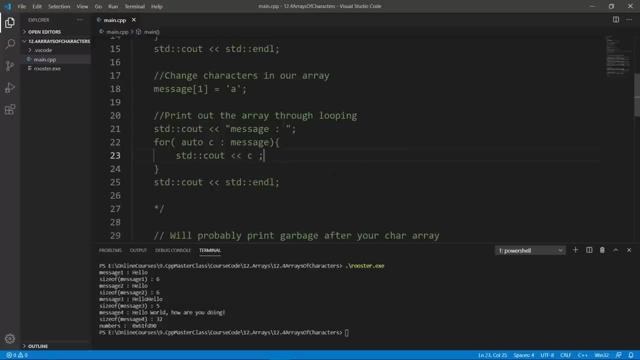 you need to be careful about in order to be able to print them out. so let's go ahead and print this out, and we're going to try to cover those in this lecture. we are going to stop here in this lecture and the next one we're going to try and look at array bounds. go ahead and finish up here. 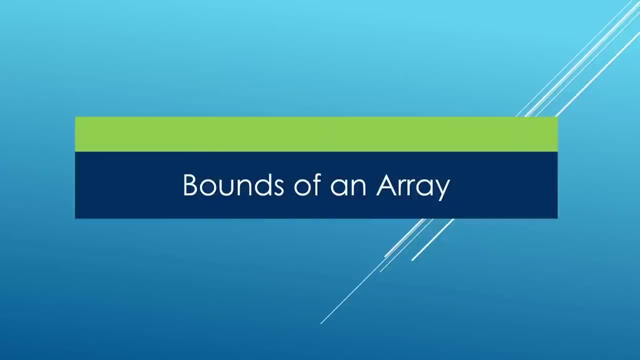 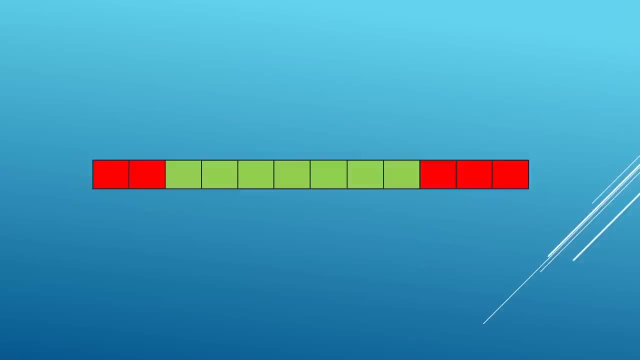 and meet me there. in this lecture we're going to look at what could happen if you try to manipulate data out of the bounds of your array. we have seen that when you allocate space for an array, the computer is going to give you a bunch of memory locations you can use to store your data. 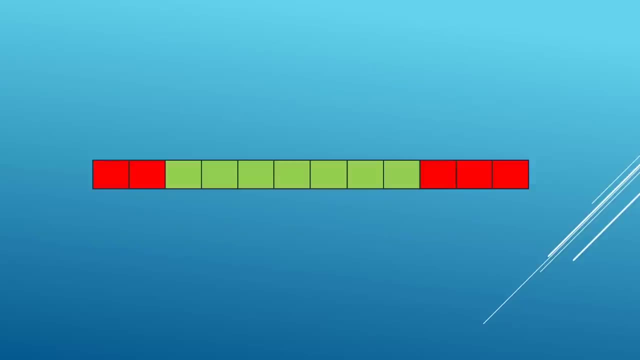 and it's going to be of the size that you have specified or that is deduced by the compiler. so here is an example of an array that is going to store seven elements and we have green slots for these elements and these are the locations we are allowed to manipulate in our c plus plus. 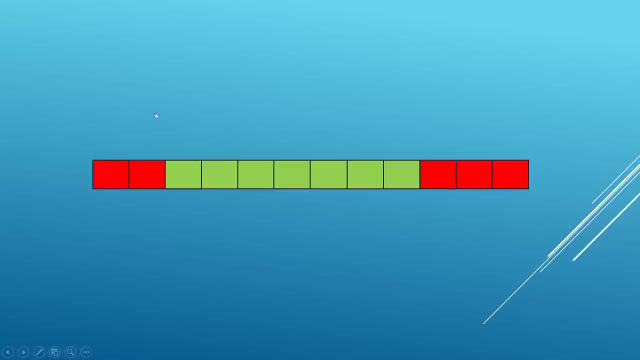 program. if we try to go over bound, for example, if we try to modify something before our array or after our array, it might be a memory location that is owned by a computer or a computer that is owned by another program. it might be a memory location that is even being used by the operating system. 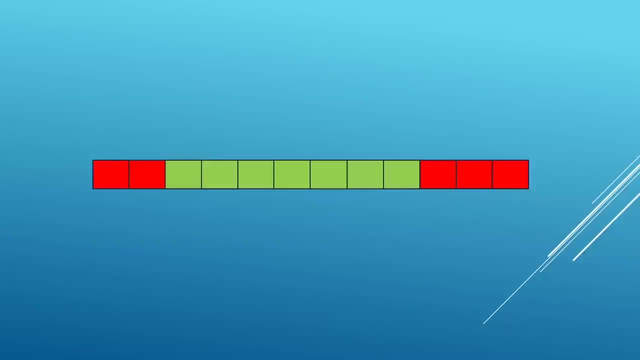 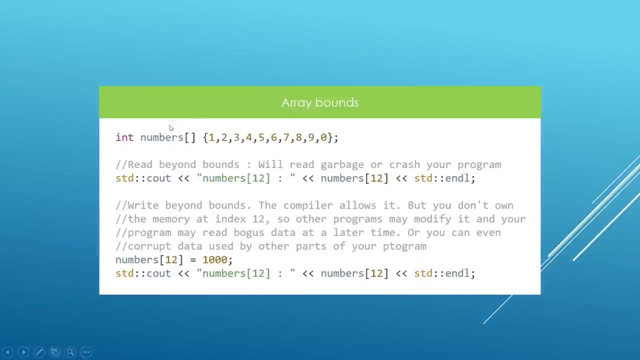 so bad things can really happen if you try to use data that is outside the bounds of your array. let's try to look at a simple example here. here we have an array called numbers. we have 10 slots inside, so we are only allowed to modify the memory locations for. 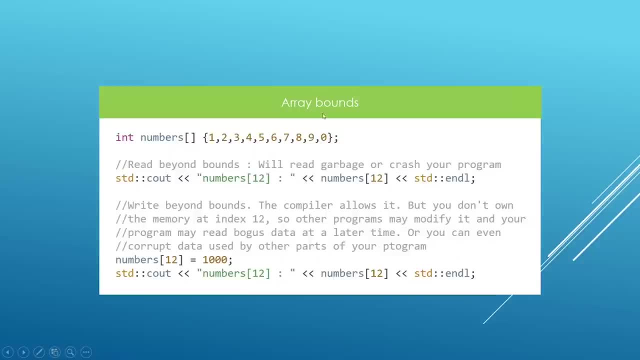 these 10 numbers and if we try to access something outside the bounds of this array, something might happen. but some people say that c plus plus is really funny because it should be stopping you from doing something like this, but c plus plus allows you to do this. if you look at code here, we have an array, we have 10 elements in, so the valid. 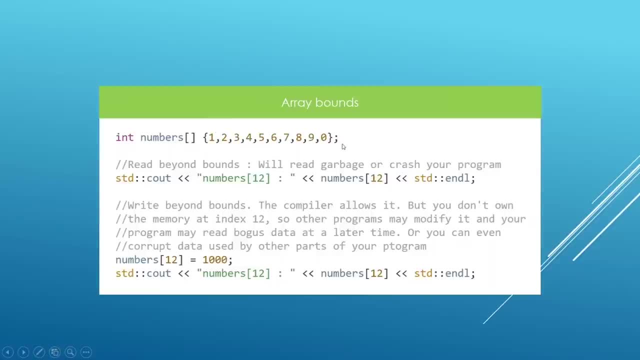 indexes we can really use are from 0 to 9.. but if we try and access something at index 12, the code is going to compile and if we run it we're going to get something printed out. but that's something really important because if we run it we're going to have something in the memory location. 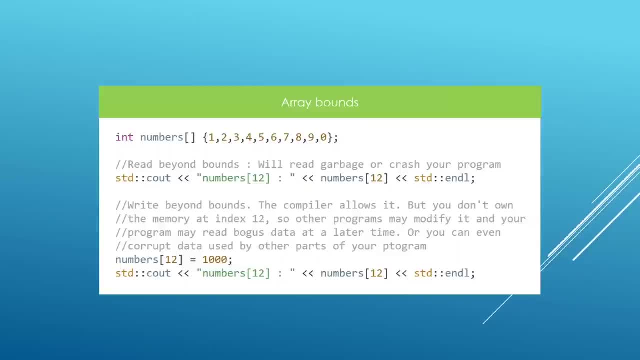 and if you try to change something it might have a different location. so you might go back to the previous example and say you just changed the memory location of the program and this is going to give you garbage data. or you might be even trying to read some restricted memory and your 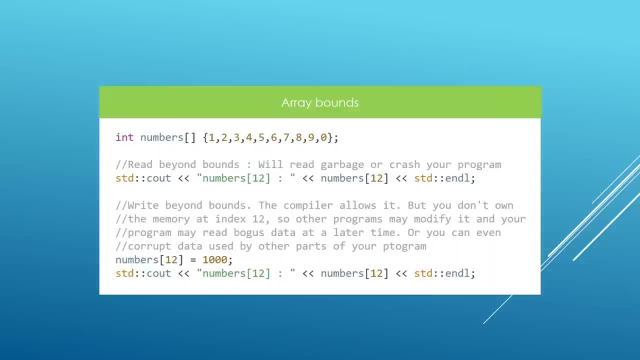 program is going to terminate immediately and we're going to say that it has crashed. if you try to write over bounds, the compiler is also going to allow it, but you don't own the memory, so data that is owned by other programs, and you might imagine how bad that really is. so the message here: 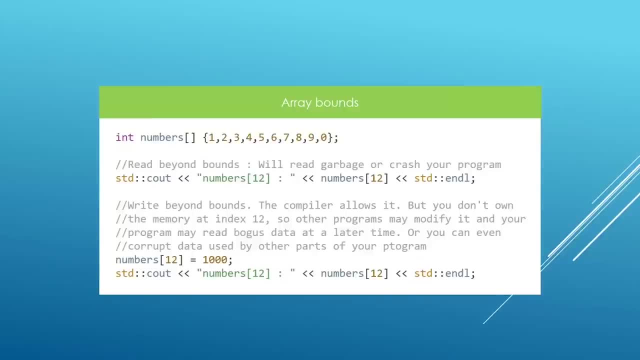 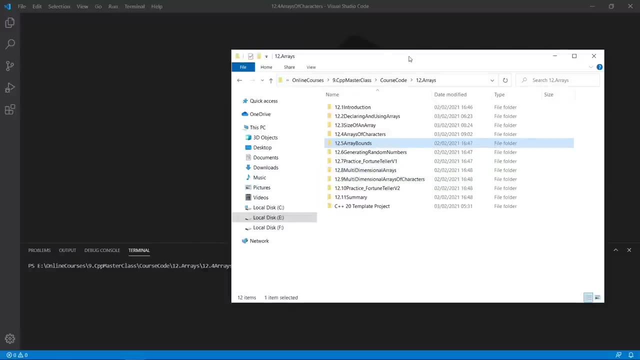 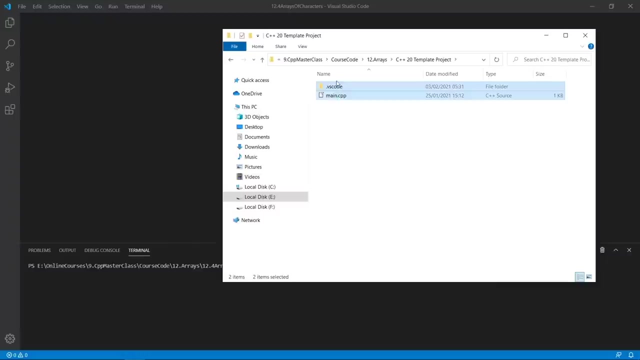 is: don't go over your array bounds, and you're going to be playing in the safe zone. let's head over to visual studio code and play with this a little bit. here we are in our working directory. the current project is array bounds. we're going to grab the template files and we're going to 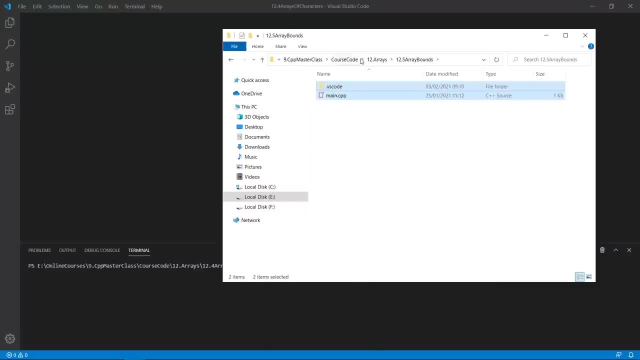 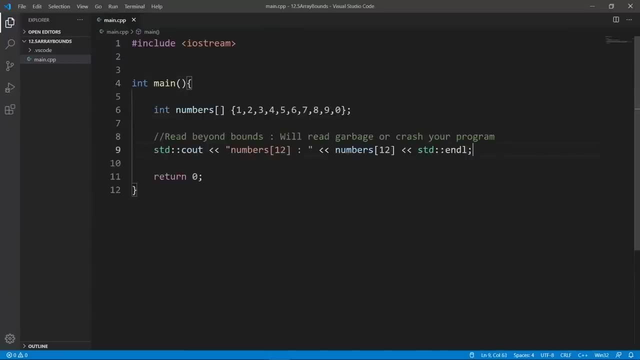 put them in place and we're going to open this up in visual studio code. we are going to declare an array and try to read beyond the legal bounds of our array. so let's try and bring up a terminal here and we are going to build this with gcc. the world is going to go through. you're not going to. 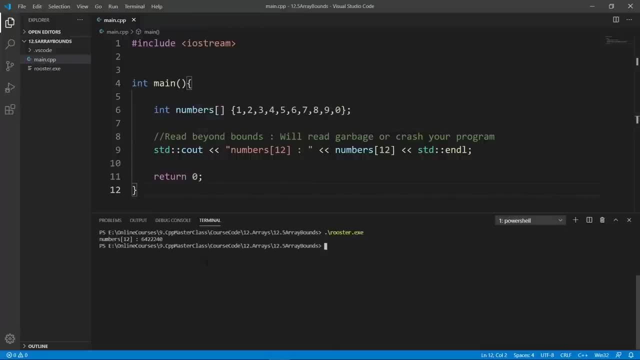 get a compiler error. but if we run this, we can really get anything. and you see, we have a number. we don't really know what it means, and this means that you have raid out of the legal bounds of your array, and c plus plus allows you to do this, and the reason they do this is because they expect you, the developer, to know what you're. 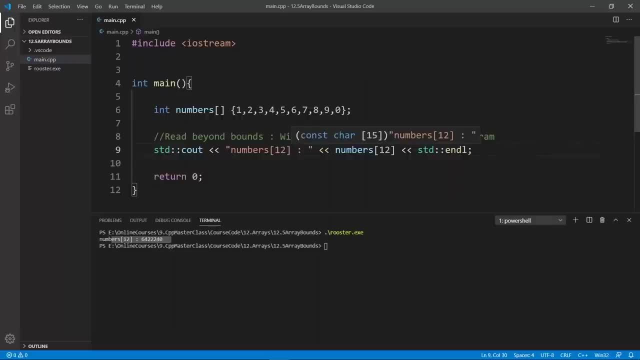 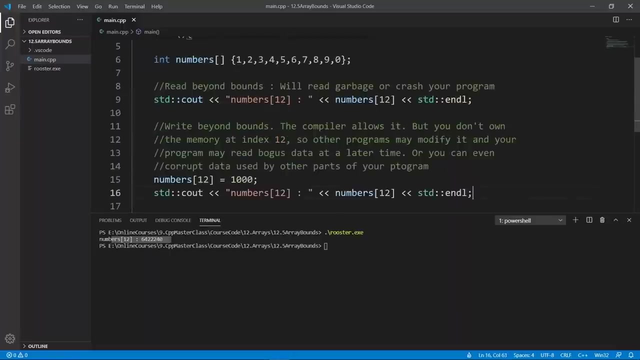 doing when you try manipulating things like array, and now you know this. and be careful when you are working with arrays like this, so don't go over, bounce. that's the message. we may also try to modify data beyond balance, so let's go down and put in the code to modify things, and i have put a clear message here as. 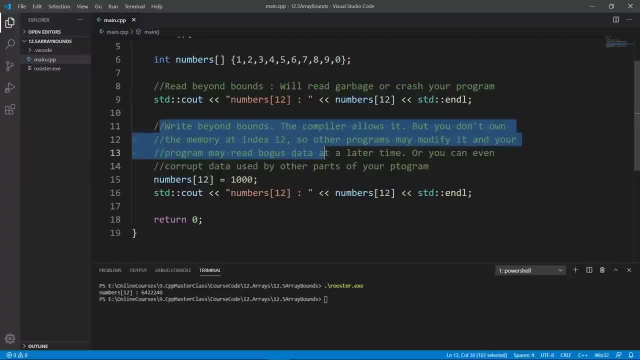 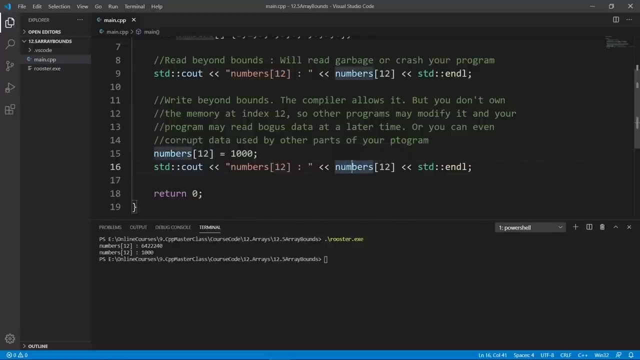 a comment to let you know that this is really something you should be very, very careful about. so we're going to try and change that number to 1000 and we're going to try and print it out and see what we get. but this memory location at index 12 is not something we own, so other programs might. 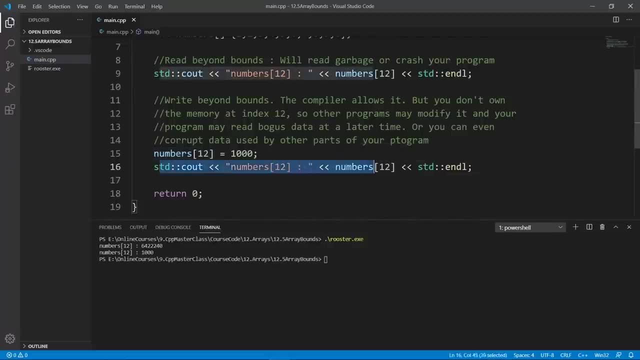 come and write to this location and if we try to read from it again, we might not get what we put in here. even worse, this memory location might be owned by other programs and if they read, they're going to get what they didn't put in. they're going to get what you. 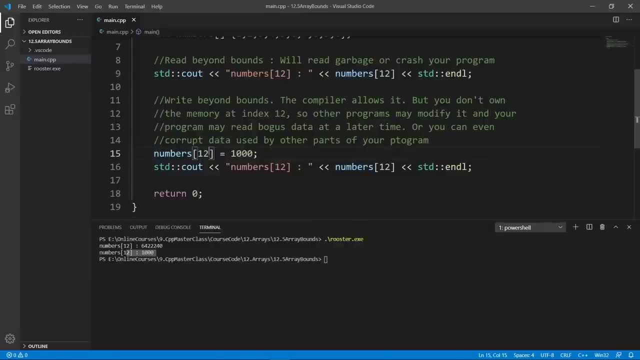 put in- and this is something bad. we might try and really go crazy with us. let's put in a really huge number and see that we can do that. this is a good way to learn, by the way, it's going to compile, and let's try and print what we have in there and we're going to say this location here. 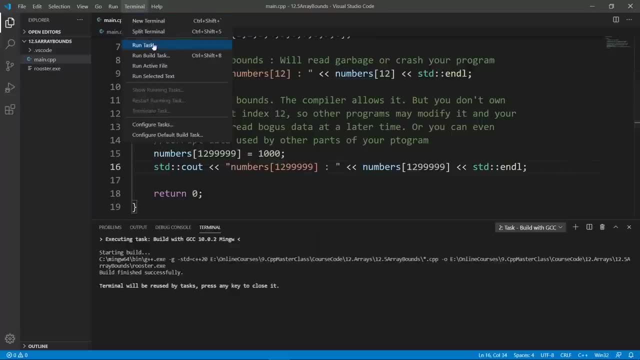 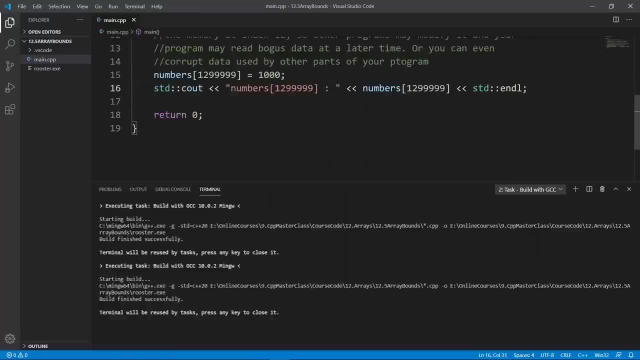 and that's what we're going to say here, and we're going to build again. the world is going to go through. you see that we are doing something really crazy. our array has 10 elements, but we are trying to modify something 1 million memory locations away, and this is really crazy. and c plus plus. 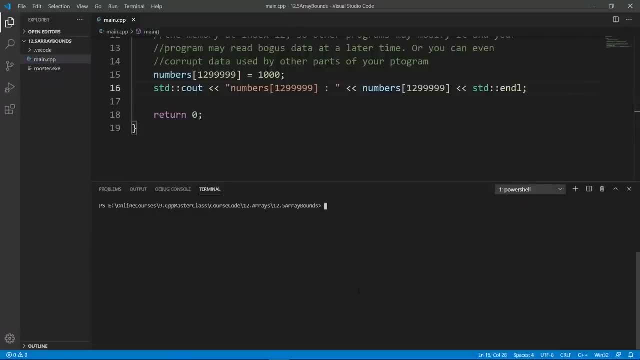 allows you to do this. so let's clear and run the web world. let's make sure we have world. so let's build with gcc and clear and run roaster. our program is crashing because we are trying to access something that isn't really ours. and you see, it has crashed okay, for example, if we have something printed out. 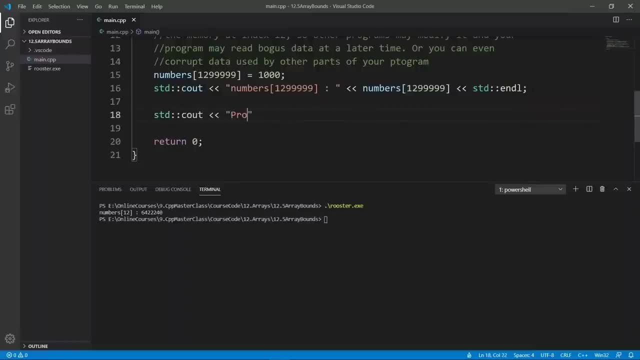 after this, let's say std program and then, so that you can see it is really crashing- and say std ndl. this statement here is not going to print because once we hit this location, we're going to try and modify it to a different location, and we're going to modify it to a different location. 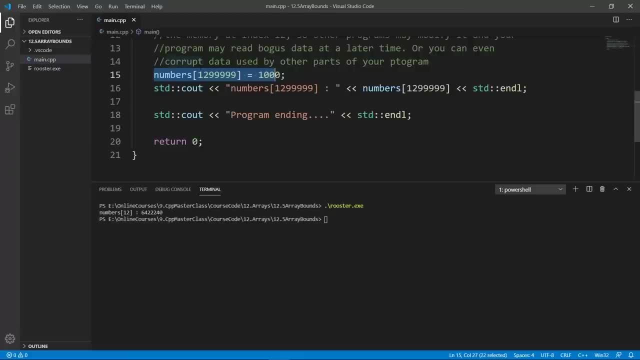 and the program is not going to be able to do that, it's going to crash. the operating system is going to notice that we are trying to do something crazy and it's going to say: this program is really crazy, it doesn't know what it's doing. i am going to kill it and it is going to 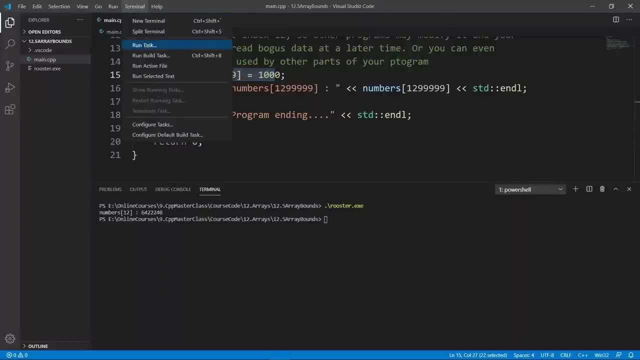 stop. that's basically what is happening here. so let's weld again with gcc and we're going to clear. let's clear and run rooster. you see that it's going to try and do this. it's going to try and put a value in here. the program is going to end here and this is really bad because memory locations. 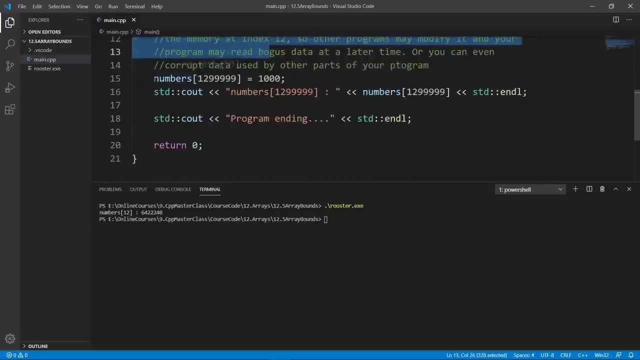 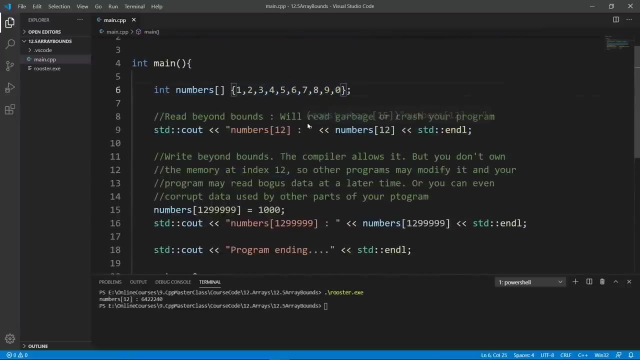 you have allocated for before here are not properly released and returned to the operating system, and this is something really bad. so the message is: don't go over bounds. make sure you are working within the legal boundaries of your array. welcome to this new chapter, and we are going to be talking. 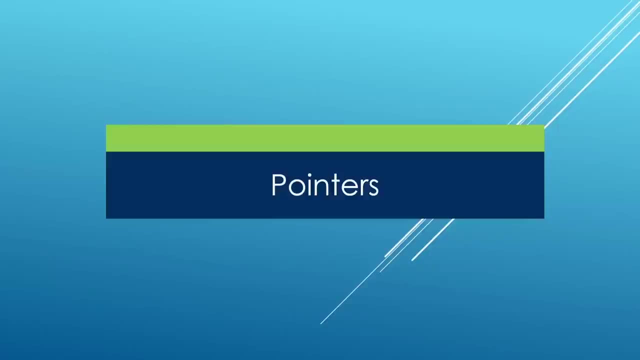 about pointers. pointers are one of the key features here. we are going to be pushing theseひ power trays in in order to tell us what to do next in enough minutes. this is just the basic example of how to its outlook, and then this is what i'm going to be talking about now. first two in this chapter. 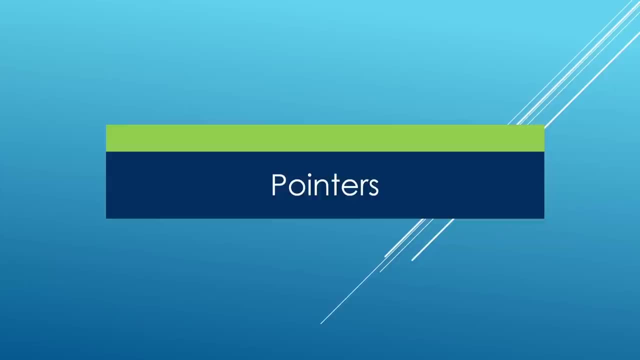 so we are going to focus mentally on the required parameters, not going back to this frame. we are going to take a look- one of the important topics in C++ and they allow you to do some of the things very conveniently, and we're going to be learning about all those tricky things you can do with them in this chapter. 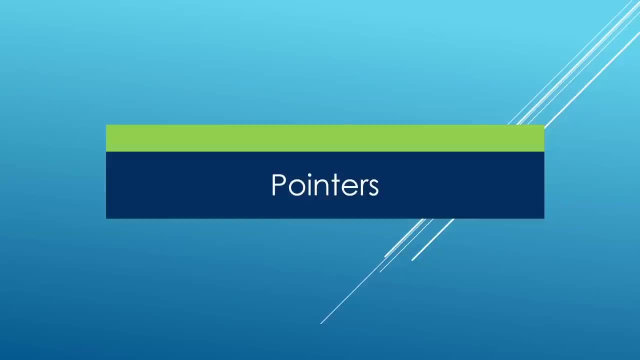 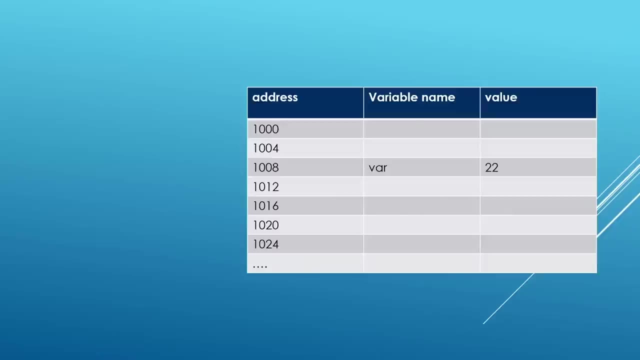 But now I want you to have a basic understanding of what a pointer really is. So far we have been working with variables like this: We set up a variable in our C++ code, We get to a point where we put a value inside that variable and we could use it. For example, we could print it out on: 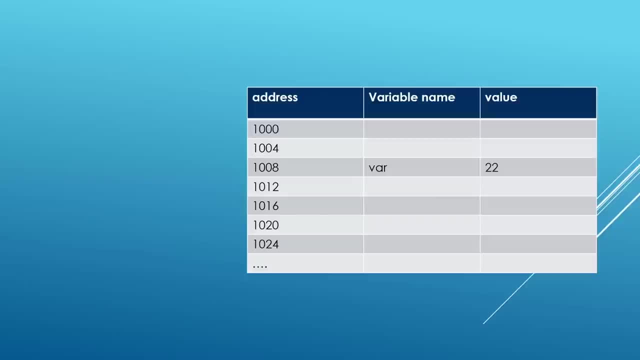 stdc out, or we could even store a value or assign another value to the variable. We've been doing that quite a lot. but there is a point we haven't really been talking about. Those variables have an address in memory and here, for example, you see that our var is stored at location 1008.. 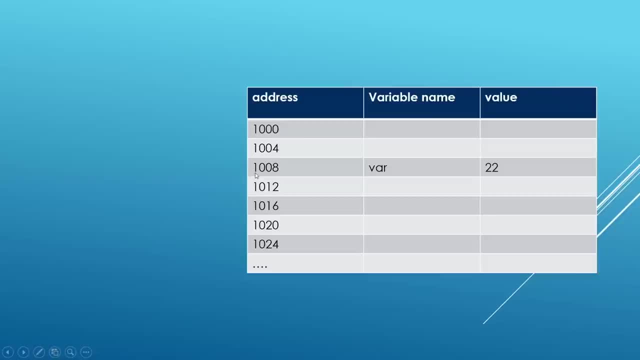 Of course this is a simple example I came up with, but I hope it drives the point home. All the variables you use in your code have some kind of address in memory And we can grab that address and store that in a special kind of variable, which is really a. 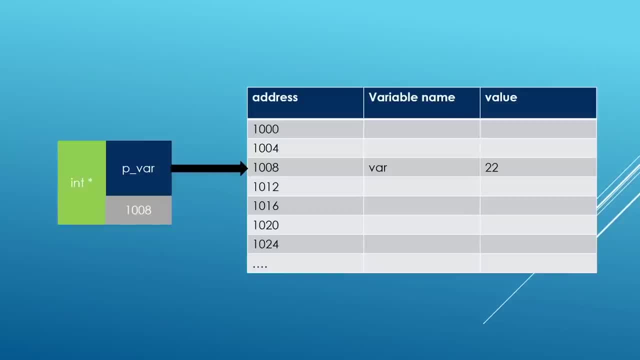 pointer. So we can say that a pointer is a special kind of variable that stores addresses of other variables. Make sure you really understand this. Here we have pvar, so it is a pointer, Its type is int pointer and we denote pointer using this star symbol after our type. If you see something like: 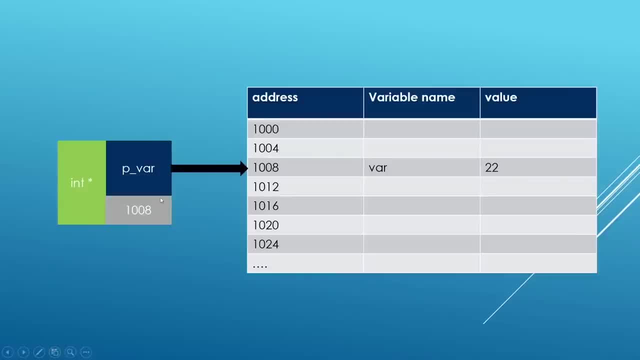 pointer to int. its name is going to be pvar because it's a variable, and its value is going to be the address of another variable. You see it is storing 1008, which happens to be the address of our var here in memory. Pointers and variables we've been talking about can work hand in hand and we're 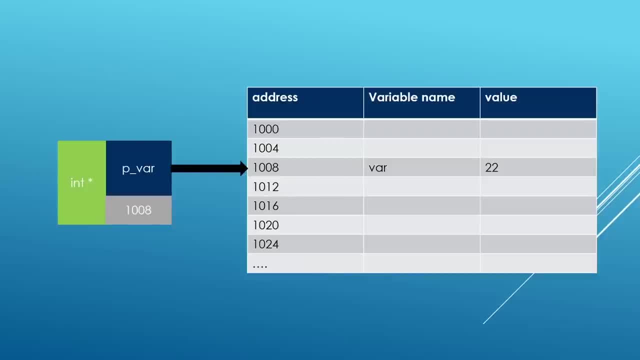 going to be seeing how this is done in the next few lectures in the chapter, but the basic idea is really the same. Here you see that we have a pointer to int, but you can have a pointer to int really to anything in your code. You can have a pointer to car, you can have a pointer to double. 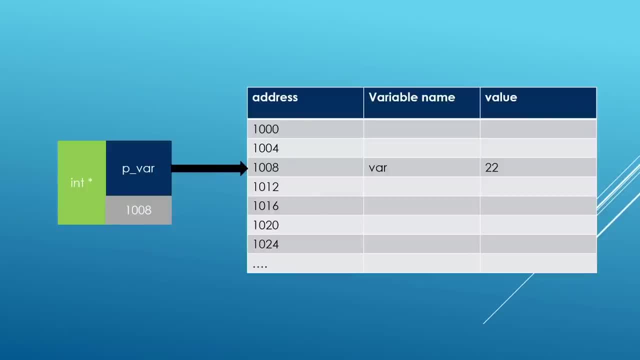 you can have a pointer to float, even pointers to custom types. we haven't really talked about now, but we will learn about them later in the course. Again, a pointer is a special type of variable in your C++ program that is going to store addresses to other variables. That's what it really is, and 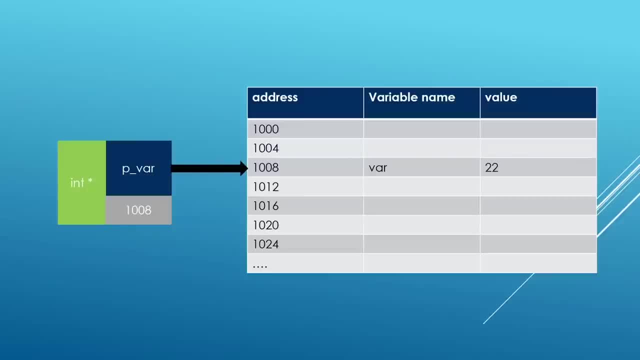 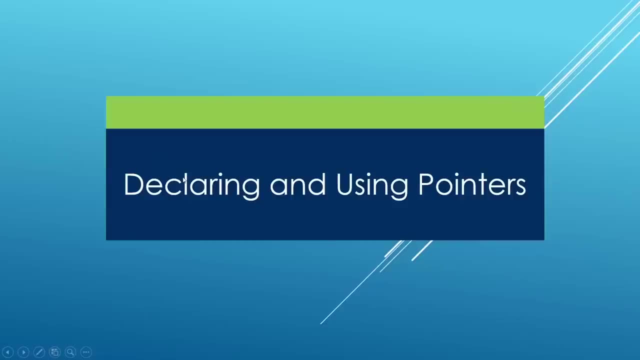 we're going to start and see how you can declare, initialize and use them in your code. Starting in the next lecture, Go ahead and finish up here and meet me there. In this lecture we're going to see how we can declare and use pointers in our C++ code. In the last lecture we said that. 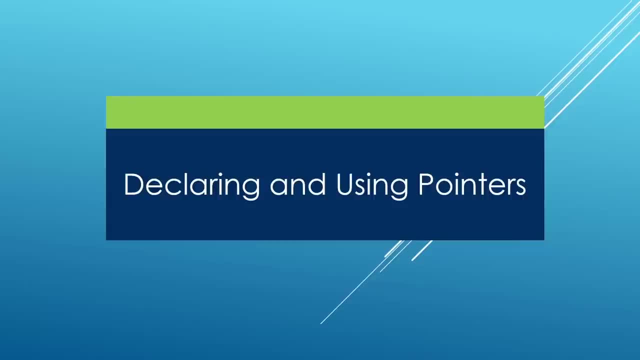 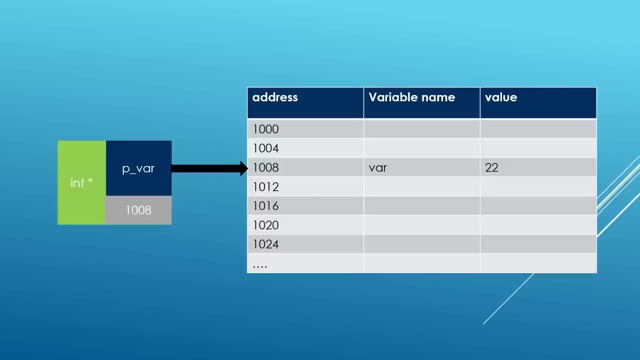 a pointer is a special kind of variable that can store addresses to other variables in our C++ code, and we have seen a slide like this to drive the point home. Now we're going to see how we can actually use pointers in our code. Here is a simple example of how we can use pointers in our code. 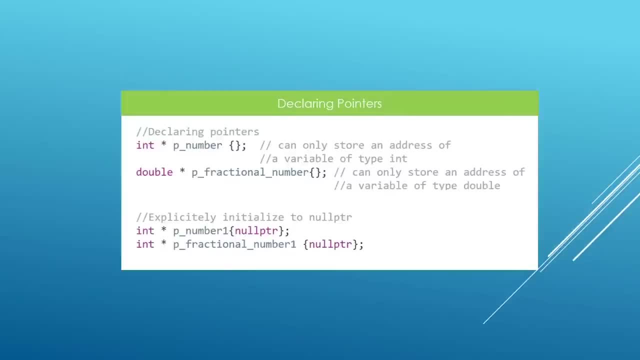 Here is a simple example of how you can declare a pointer variable. in your C++ code You say int. you put a star after the type to mean that this variable is not a regular variable like we have seen before. It is a special kind of variable that is going to store addresses to other variables. 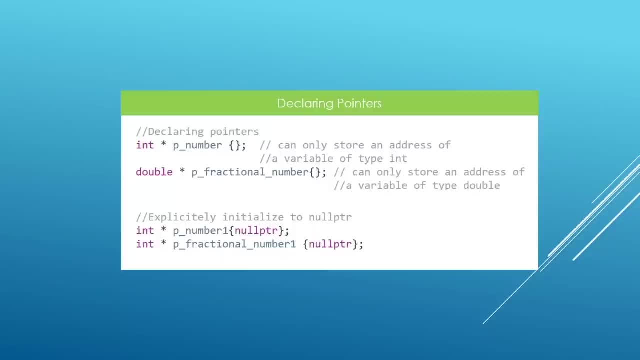 and here I have to say that you have to be really careful and only store addresses to valid types of variable in your pointer. For example, this is a pointer to int. It can only store an address of a variable of type int. For other types, if you try and put in their addresses in here, you're going to get a compiler. 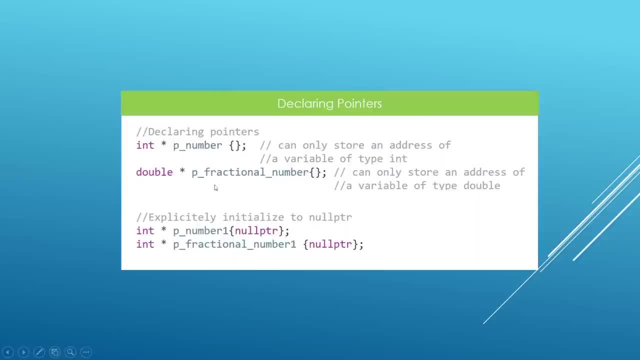 error Down here. you see, we have another example and it's called p fractional number because it's a double, and you see that our pointers here are initialized using braced initializers and this is going to initialize the pointers with a special address. that really brings the pointer to the 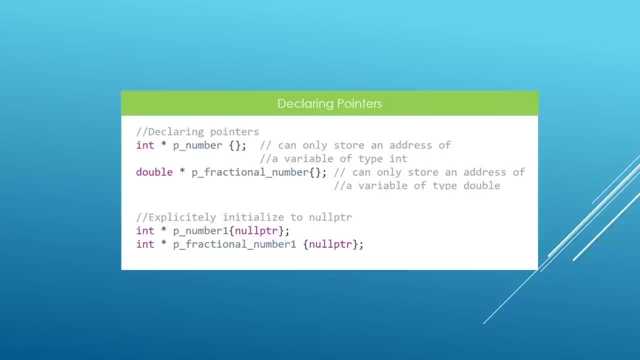 same value. So you can see that this pointer is not pointing to anything. yet You can also say that explicitly and put null ptr inside, and this is going to mean that these pointers are not pointing anywhere. You can't really use the values at the addresses where 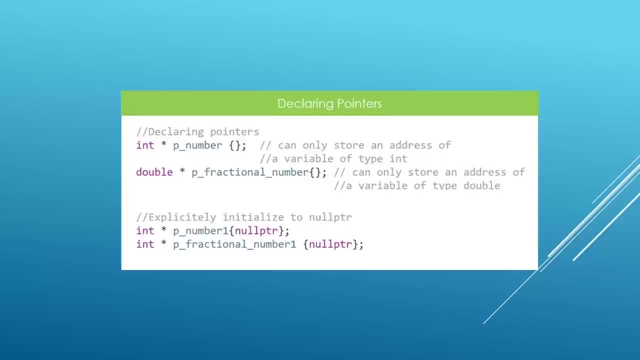 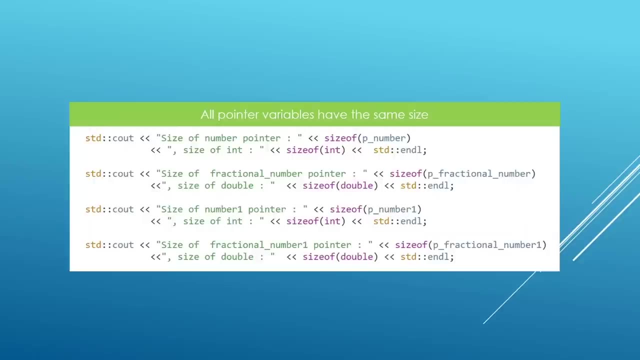 they point. This is the message here: Don't use pointers that contain null pointer. All pointers on a given system are going to have the same size. For example, if you have a pointer to int and a pointer to double, they are going to be the same size because they really store the same thing. 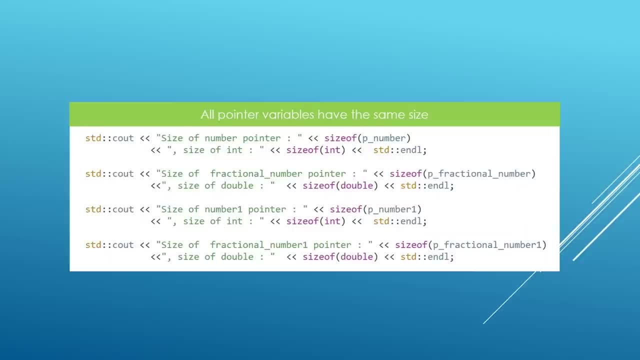 They store addresses to variables and addresses to different variables, even if they happen to be of the same type, on the same system, out of the same size. That's why all the pointers you're going to use in your code are going to have the same size, and this is something you should keep in mind. 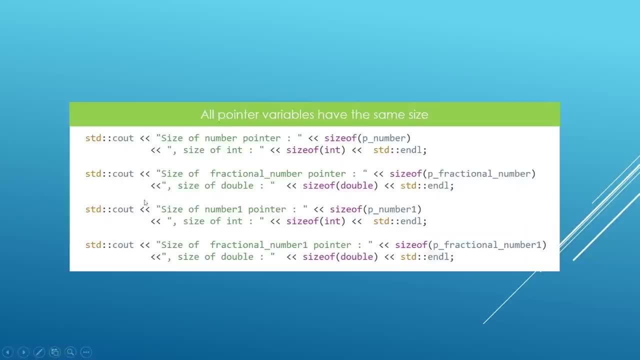 And here is a simple example to really play with that. We have a size of int printed out. We have a size of our pointers printed out. We have a size of our pointers printed out. We have a size of our pointers printed out. And we're going to compare these things when we get to Visual Studio Code in a 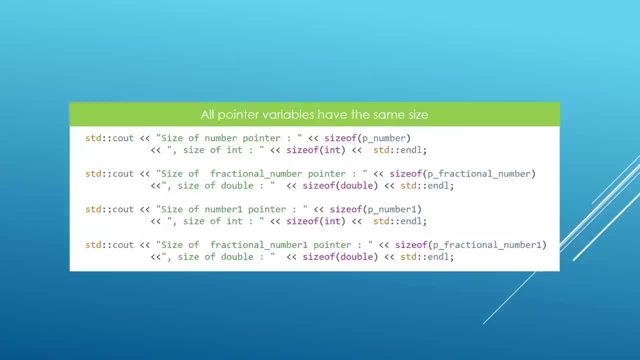 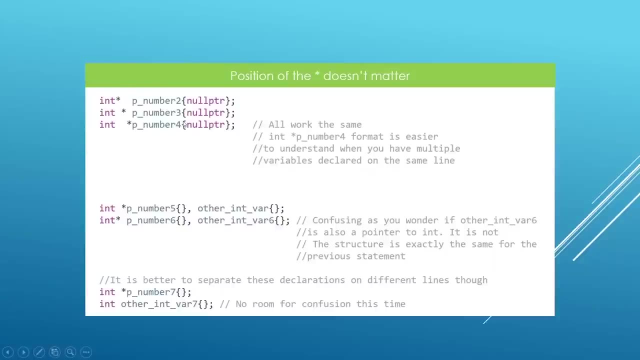 minute And you're going to see that all pointers are of the same size. A question I get from many people is if the position of this star symbol really matters- And I have to break it to you, It doesn't, But I prefer to put it on the left. Some people prefer to put it on the right, But 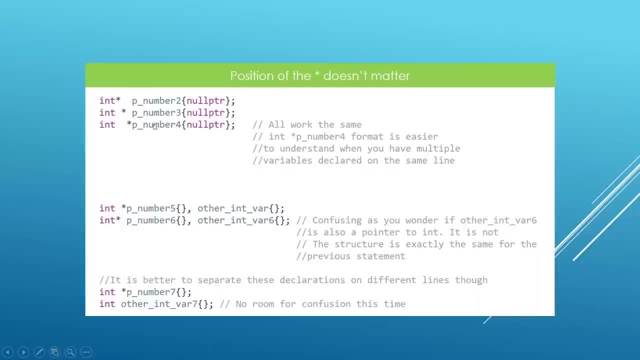 definitely don't put it in the middle. I've never seen anybody do this, But it's going to work. It's another thing I see people do which is really confusing is to declare your pointers on the same line and do a comma like this. This is really going to be confusing, And now I want you to guess and. 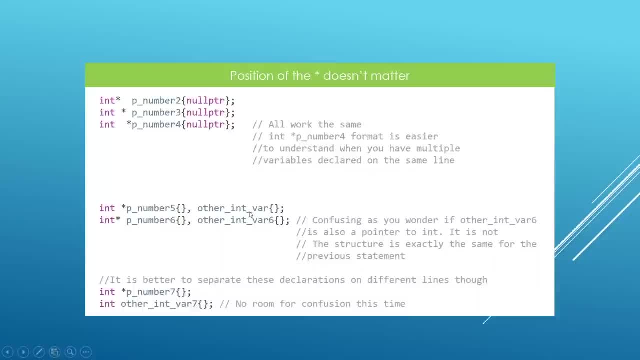 see what is happening here: Is either int var a pointer, or it's a regular int. I want you to keep this in mind. I'm not going to tell you We're going to try this out actually in Visual Studio Code and we're going to figure this out together. But now I want you to try and think about it. 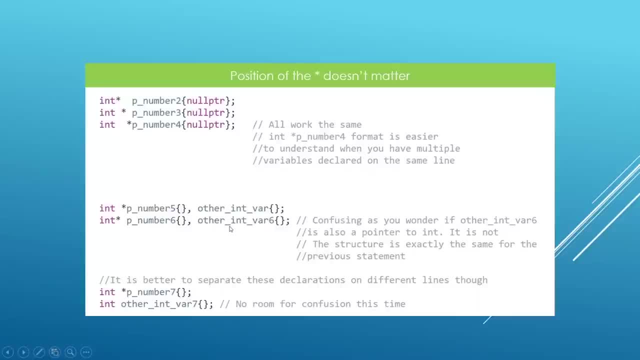 Leave this question unanswered, and we're going to answer it in a little while, But for now don't really do this, because it's confusing and it's going to make your code less readable. If you have to do something like this, make sure you just put them on different lines. 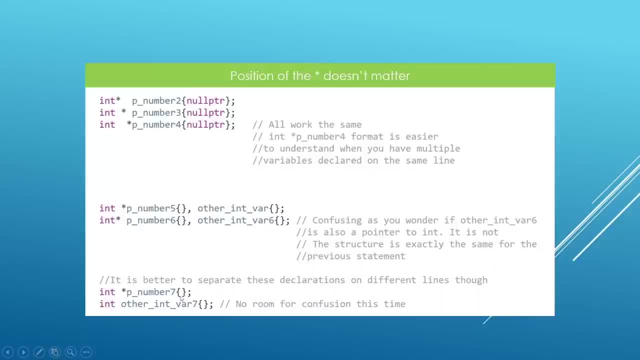 and it's not going to be confusing. For example, if you look down here, you're going to know that p number seven is a pointer. Other int, var, is a regular int and there is no room for confusion this time. Use code like this and don't put things on the same line. 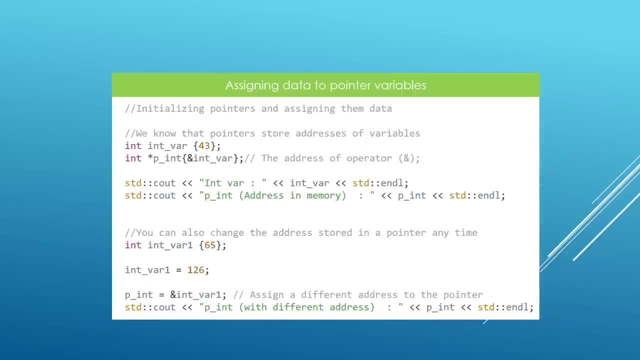 Like we have on top here. Okay, now we have seen that we can declare and initialize pointers with null pointer. Now is the time to see how we can put actual data in those pointer variables. Here we have a variable which is called int var. It is of type int and its value is a 43.. We can also 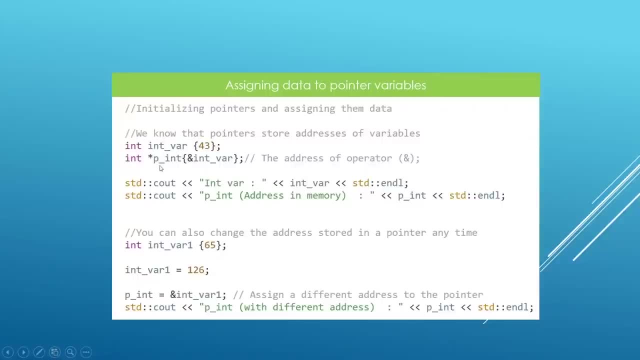 set up another pointer variable, int pointer. Its name is p, underscore int, and we can initialize it With the address of another variable. and here is a new operator we haven't seen before. This ampersand variable here really means the address of this int variable. That's what we mean here. 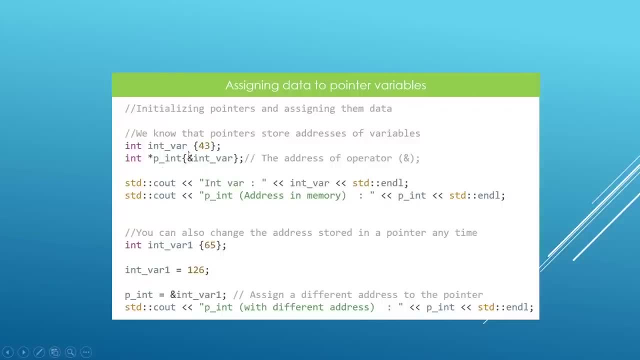 So we're going to initialize this p int variable with the address of int variable. and this is how we do it. If we go down here, we print int var, We're going to get the value printed down. If we print the pointer directly, we're going to get the address of this little guy. 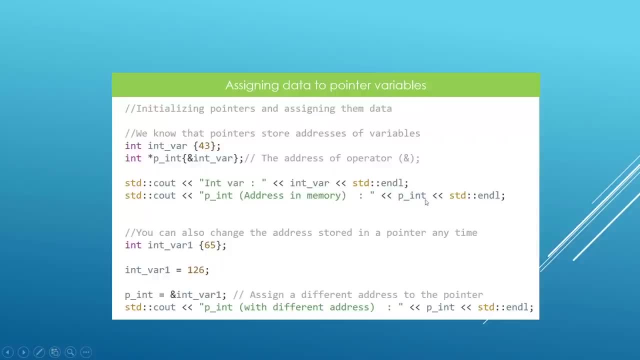 printed. Okay, so this is how you can store things in your pointer variables, and what you have to store in has to be an address of another variable. Down here you see we have another variable called int var 1.. Inside we have a 65 and if you go down here you see that we are storing something else. 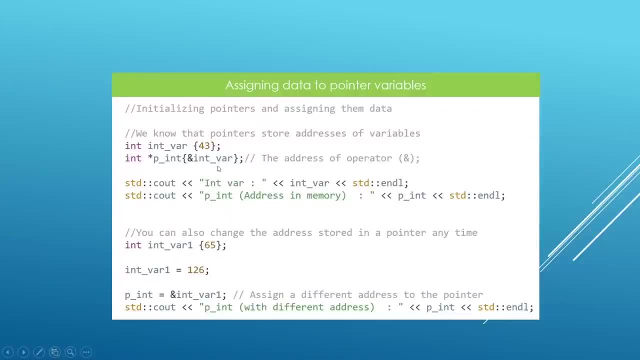 in our pointer variable. here We had in the address of int var. Now we are putting in the address of int var 1 using an assignment. So we're going to put in the address of int var 1.. We're going to put in the address of int var 2.. We're going to print it out. We're going to put in an. 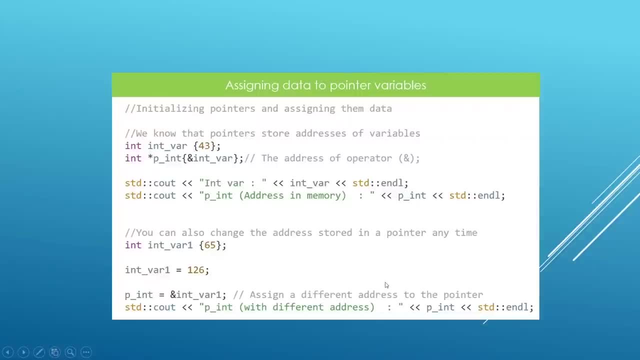 assignment operator and this is something you can definitely do. It's legal C++, It's going to work. If we print it out, we're going to get a different address printed out. This is how you can store values in your pointer variables. Again, you can't cross assign before different pointer types. 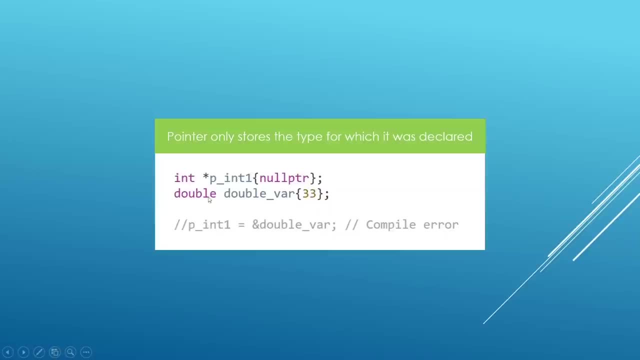 Here we have an int pointer which is called p? int 1 and we have a double variable. It's called double var. We can't take the address of double var and store that in p? int 1.. This is going to be to be a compiler error. the variables whose addresses you store in pnt1 have to be of type. 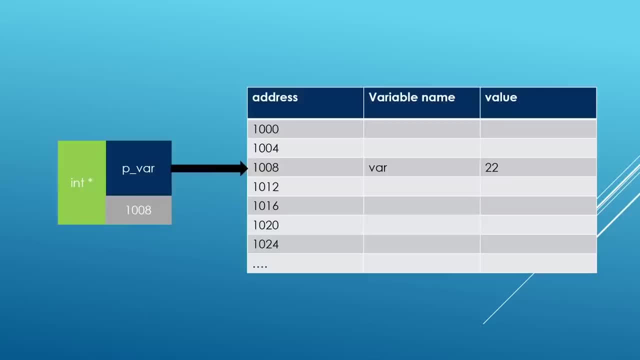 int again. the basic idea is that a pointer is really a special kind of variable that is going to store addresses to other variables and if your pointer is a pointer to end, the variables whose addresses you can store in this pointer to end can only be ends if you try and put in doubles. 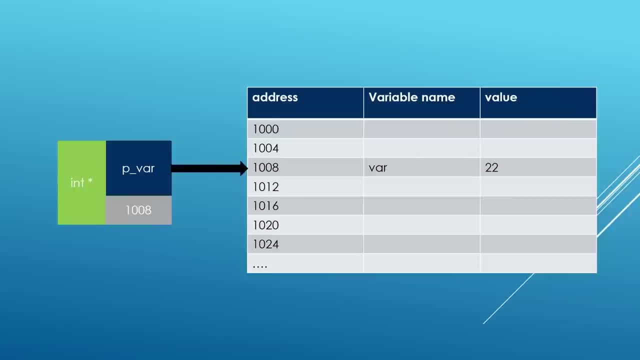 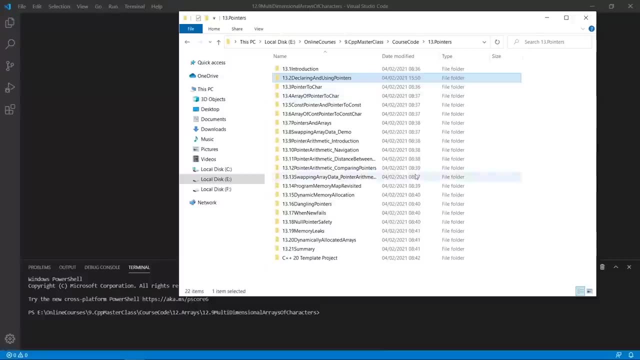 you're going to be in trouble. you're going to get a compiler error and it's not going to work. now we're going to head over to visual studio code and actually play with these things. here we are in our working directory. the current chapter is pointers. the current lecture is declaring and using pointers. 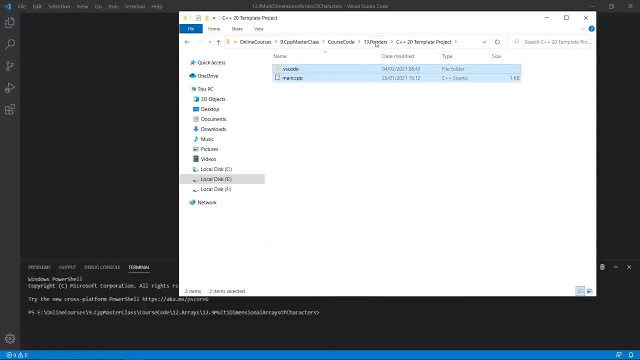 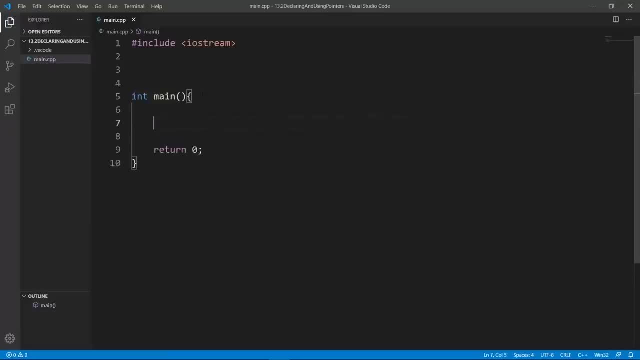 we're going to grab our template files and put them in place, so put them in our project here, and we're going to open this in visual studio code. the first thing we're going to see is how we can declare and initialize pointers, and we're going to use a pointer to end as a first example. we're going to 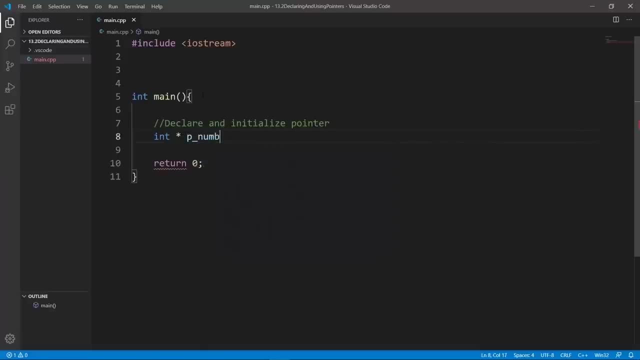 set up an int pointer and we say int star, we're going to give it a name, we're going to call this p number and you can leave it like this, uninitialized. but it is really advised to always initialize your pointers. so we're going to do that with a braced initializer which is going to do: 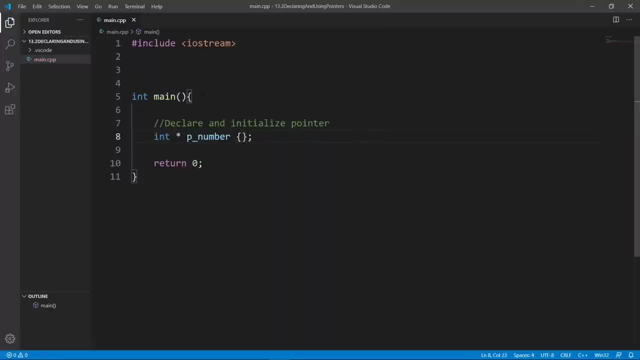 that for us, this is going to implicitly initialize it with a zero equivalent of pointers, and that happens to be null pointer, so we'll initialize. okay, see, this is what we're going to initialize with no pointer. we say null ptr, and this is how you should do things. we can also do a pointer to double, why not? let's do. 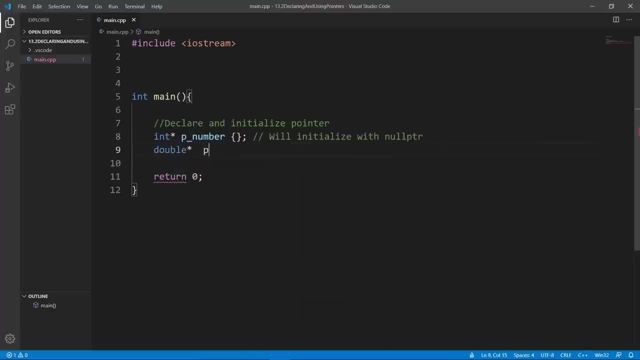 double pointer and we're going to say fractional number pointer to fractional number, and we can also initialize this with null pointer. implicitly and once you do this, the program is going to be legal. if we try to weld it with gcc, like we always do, the build is going to be good, but we don't. 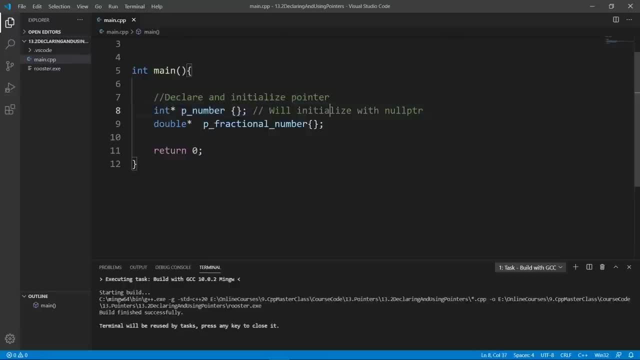 really have any useful thing we can see if we run this program. we are just getting started. we will get to see things later. for now, just understand that p number is a variable we have in our code. this variable can only store addresses to other variables that happen to be of type. and if you try, 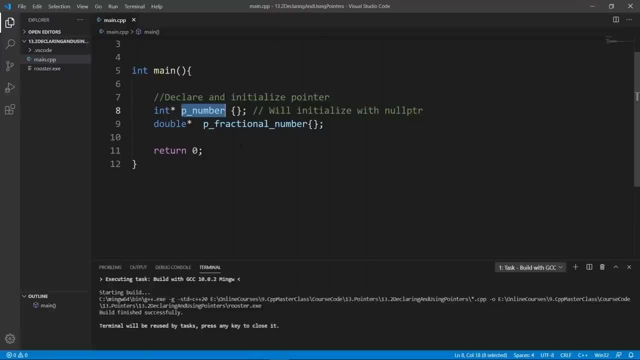 to store addresses to other variables that are of type double, for example, or float, you're going to get a compiler error. you shouldn't do that. the same for p, fractional number: it can only store addresses to other variables which happen to be of type double. keep this in mind. we can also 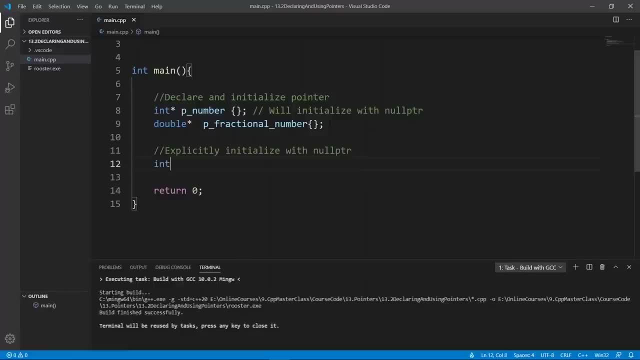 explicitly initialize with no pointer. so we can say int pointer and say p number one- why not? and we're going to explicitly use no ptr like this, and this is going to work as well. we can also say p fractional number and say one- why not? and say now ptr. 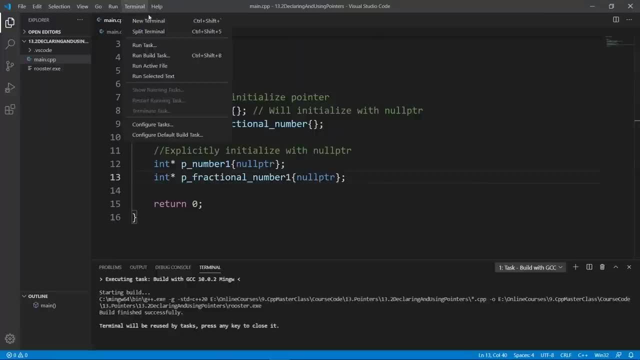 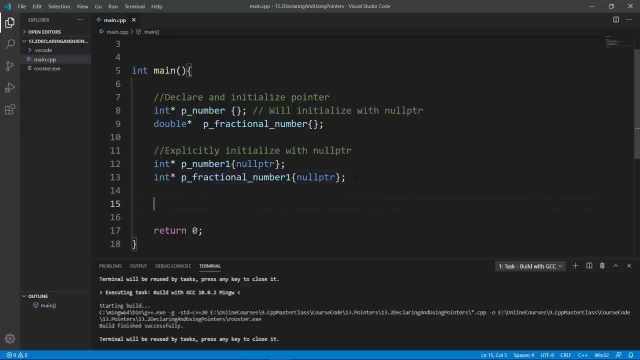 this is going to work. this is something you can do. you're going to see that if we compile this, the compiler is going to be happy with this. the build is good. okay, now you know how you can declare and initialize your pointers. now we're going to see that pointers to different variables. 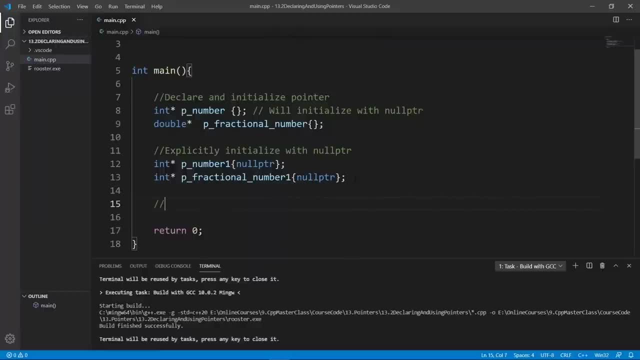 are actually of the same size on whatever system you are working on. it's not consistent across operating systems or refund systems, but it is guaranteed to be of the same size on the same machine. i am going to go down and put in a piece of code that is going: 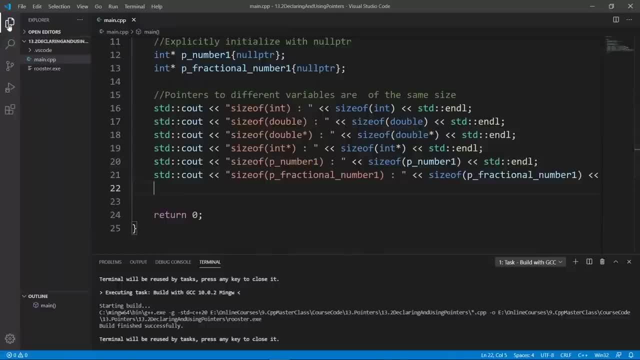 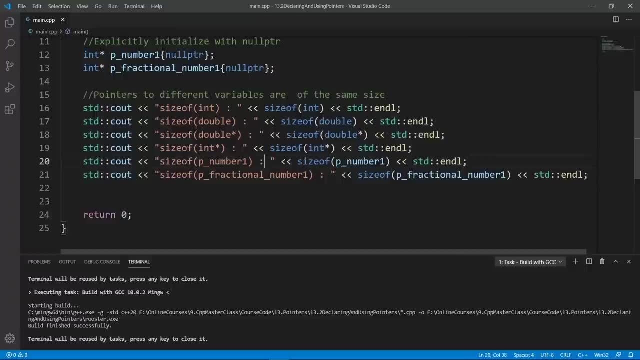 to show us all these things on the console, and i am going to click on this file icon here and give ourselves some breathing room so that we can see the entire thing here. if you look, here we are printing the size of ant. we know that this is going to be a four size of double. this is going 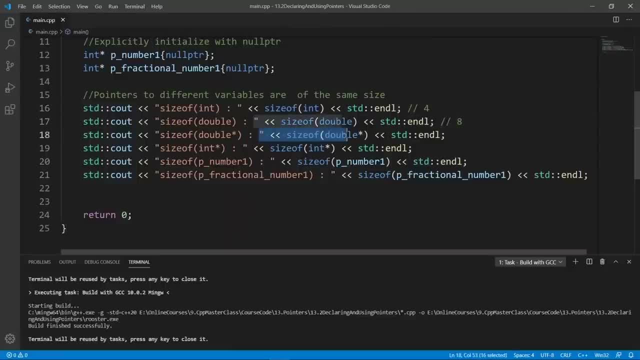 to be an eight on our system here, but we don't know what the size of a double pointer is or the size of an int pointer, and we're going to see that in a minute. here you see that we are also using the pointer variables immediately. this is something you can do. you see that visual. 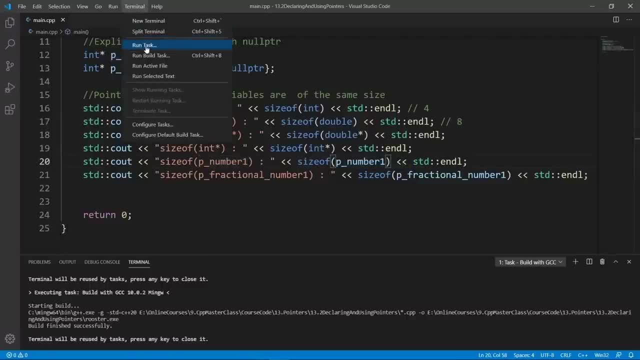 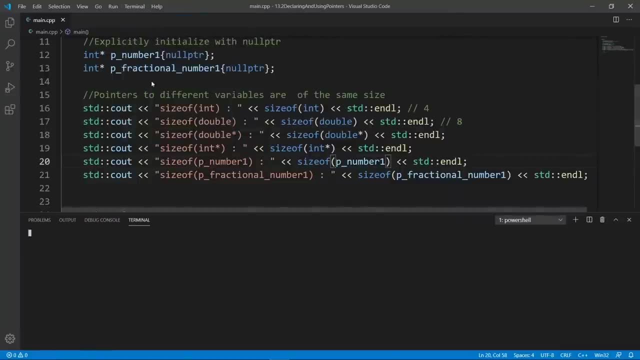 studio code is not complaining and we can go on top here and weld with gcc. let's do that. the world is going to be good. now we can open up a terminal and actually run this program here. we're going to clear. if we do there, we're going to see that in our directory here. so you see that we. 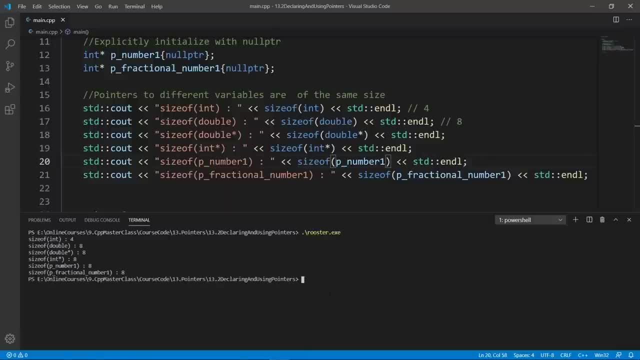 have roosterexe and we can run this and it's going to say: size of ant is four, size of double is eight. this is expected, but pointer types are of size eight. on my system they occupy eight bytes in memory, so it doesn't matter the type we are pointing to a pointer to. it is: 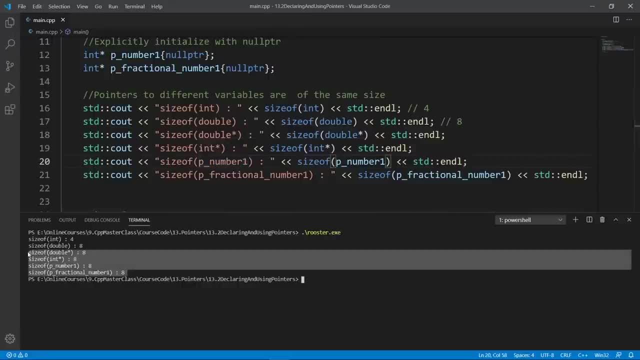 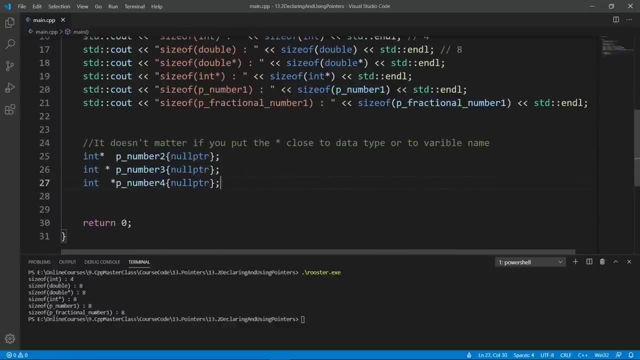 going to be eight bytes in memory. this is something you should really know and keep in your mind. another thing we have said that i want to play with right now is the location of this star symbol. some people say you should put it on the left. some people say you should put it to the 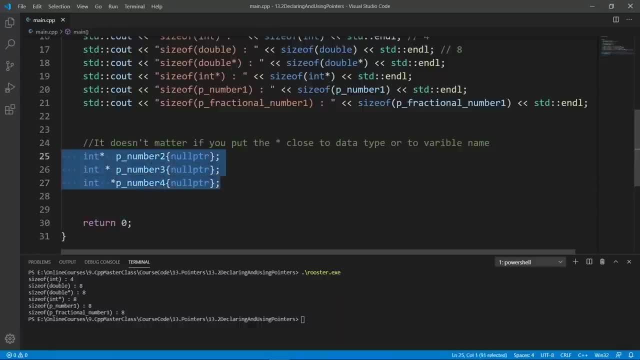 right. i don't really think any of these things matters. i prefer to put it to the left, but if you put it to the right, it's also possible. it's going to work. you see that, even if you put it in the middle here, which is really crazy- the compiler is going to take this. 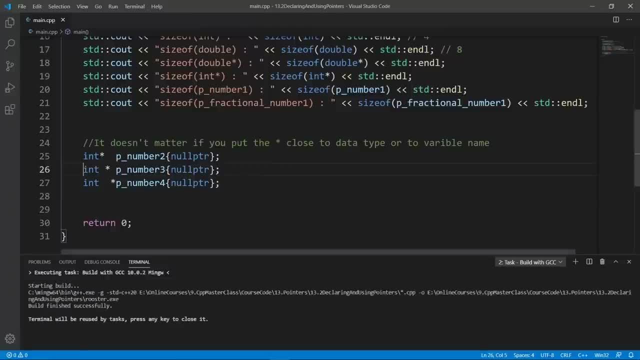 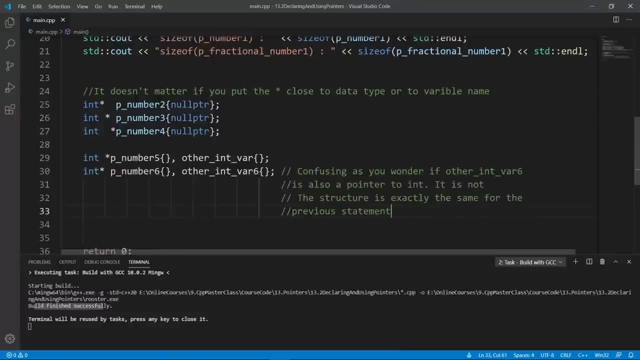 we can run the task to build this, to make sure the compiler is really happy, and you see that there's no problem. the compiler is going to accept this and we are going to build successfully. if you put your declaration on a single line like this, what is other int var going to be? is it going to? 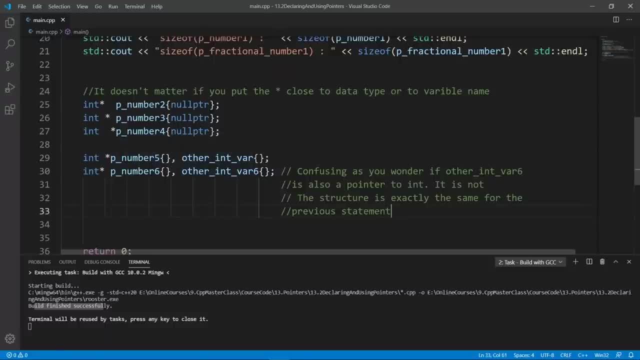 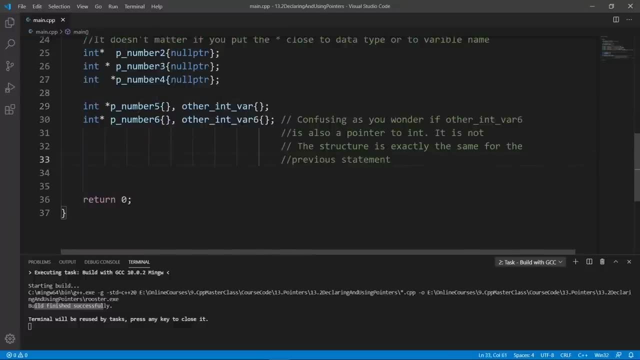 be a regular int variable? is it going to be a pointer to an? we don't really know now and i don't want to tell you. we're going to find out together. so what we're going to do, we're going to print the size of these things. i am going to 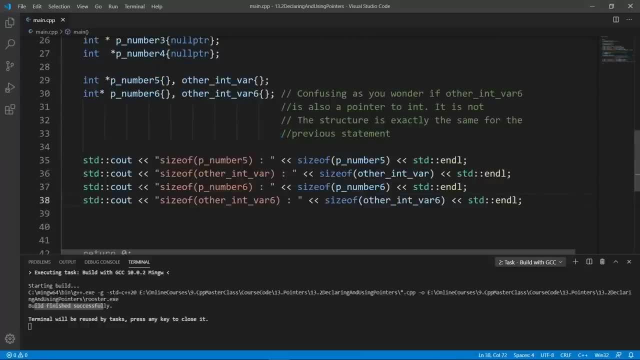 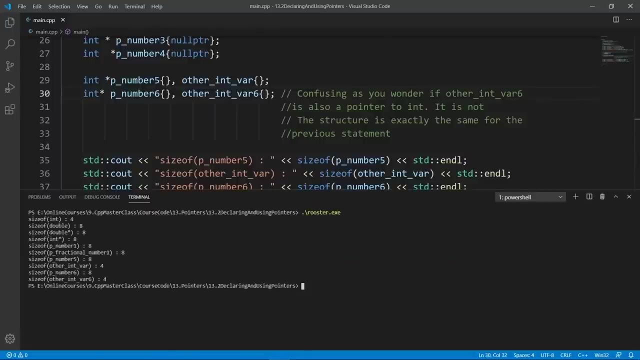 go down here and put in the code and come back in a minute. here is our code typed out and we're going to see the size of these things. what we're going to do is run the task to build with gcc, as we always do. let's clear properly and run rooster and you see size of p. number five is eight. 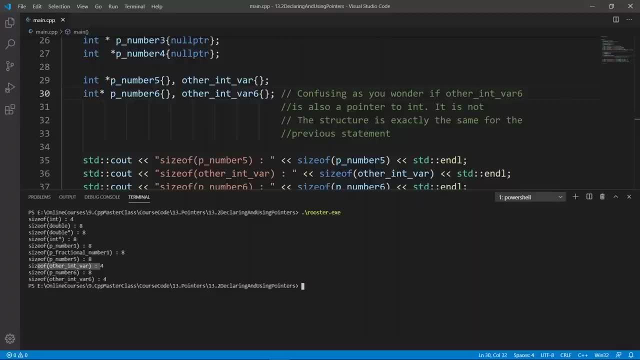 because it's a pointer. size of other int is four, and the same applies to the second line here. so from this we can tell that other int var and other int var six are not pointers, they are regular integers and this can be really confusing. so to avoid this confusion i would advise not to 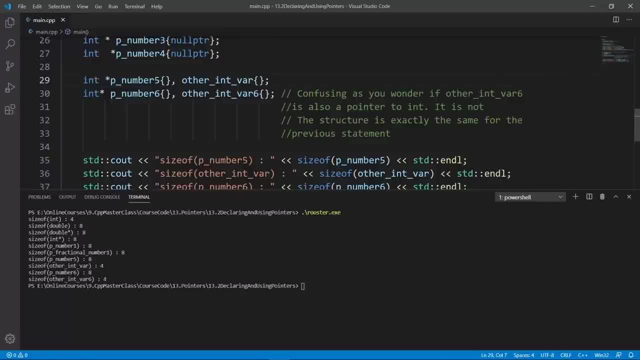 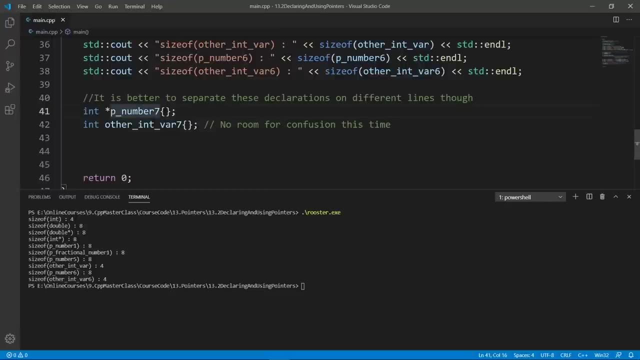 declare your thanks. when you have pointers inside like this, because that's going to be really confusing, what you can do is put them on separate lines and do something like this. so here it is very clear that p number seven is a pointer. other int var seven is a regular int variable and there is no room for confusion. 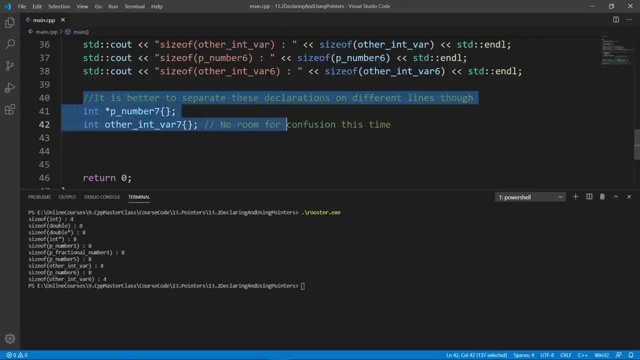 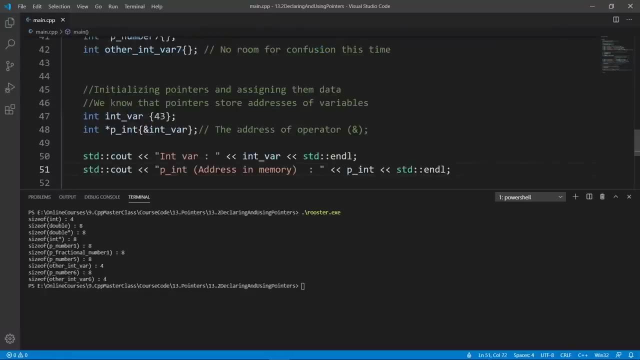 with this way of doing things. so make sure you put things on separate lines like this, and you're going to be fine. now what i want you to see is that we can actually store data in our pointers. i mean valid data, that is not a null pointer. in this case, we're going. 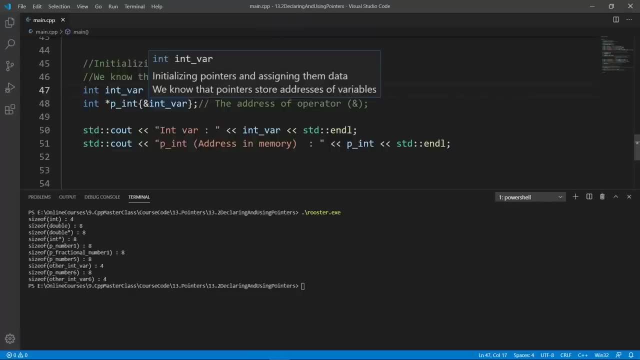 to set up a variable, a regular int variable. it's going to store a 43 inside and we're going to set up another pointer and initialize that with the address of this int variable variable and this is going to work properly. what we can do now is print the interval. we're going 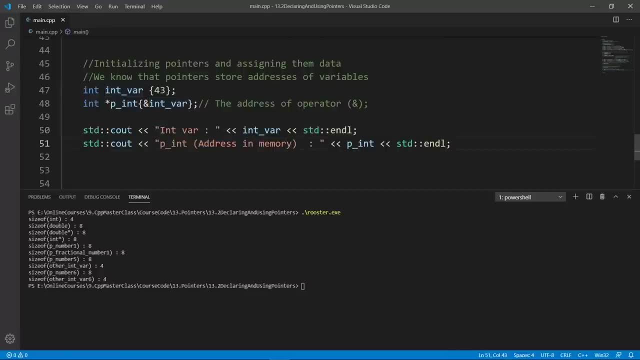 to print it out. if we try to print the pointer, we're going to get the address of this interval in memory, and this is something you need to see with your eyes. this is the first time we are printing out an address that is stored in a pointer and we're going to see that on the console here. 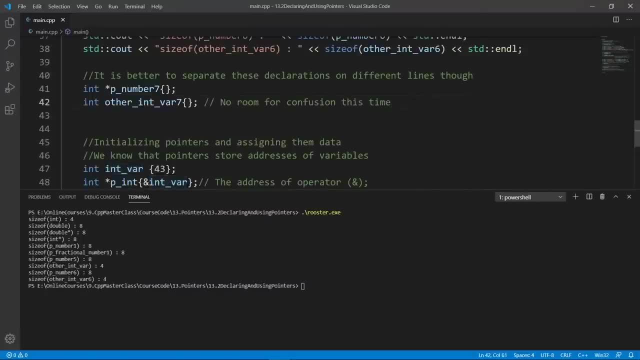 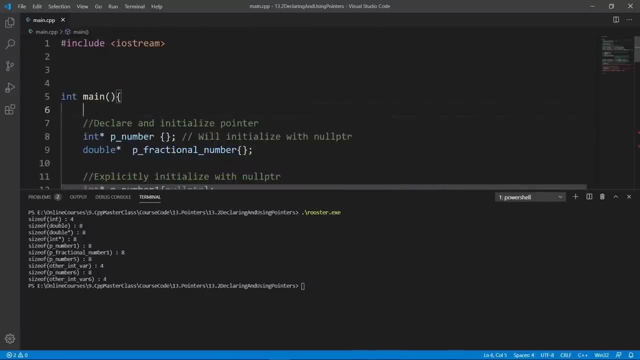 what i am going to do. before we build and run this, i am going to comment out everything we've done before, because our console is now cluttered. so let's come and comment out everything and let's go down again now. if we print, we're going to see these two statements and that's. 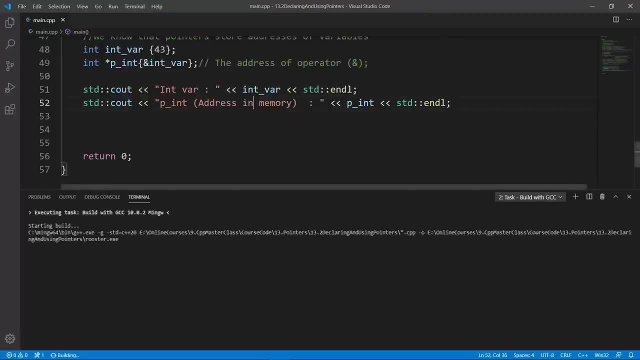 going to be easier to follow on the console here. the both is good, so we are cool. let's run rooster. and the var is 43 and its address in memory is this number. here it is in hexadecimal, so this is the address in memory and we can print that out and see what. it is okay, so this is really cool. 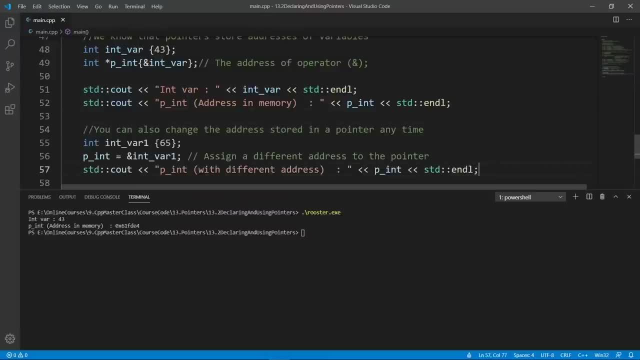 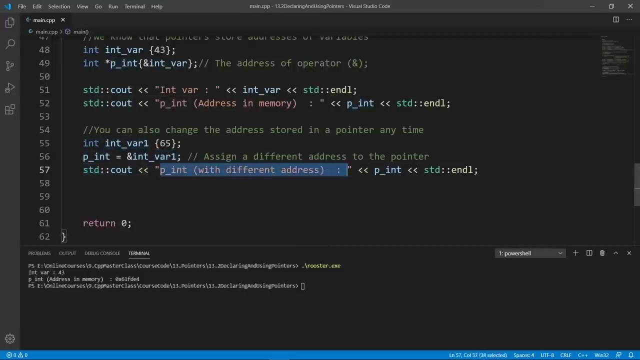 but we can also change what is stored in our pointer here. for example, we can set up another variable, call it int var one, and change p int, which is a pointer, to contain the address of this new variable. and we can do that. now, if we print p int, we're going to see that it contains. 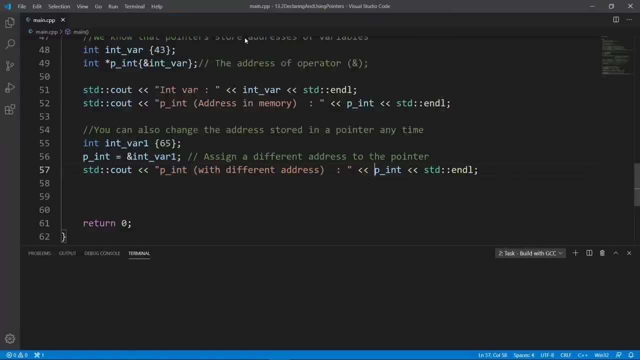 a different address and we can do that. so let's go with gcc again. we're going to go down and clear and run rooster and we're going to see that now we have a different address: the one we had ended in de4, now we end in de0. these are different addresses and we are. 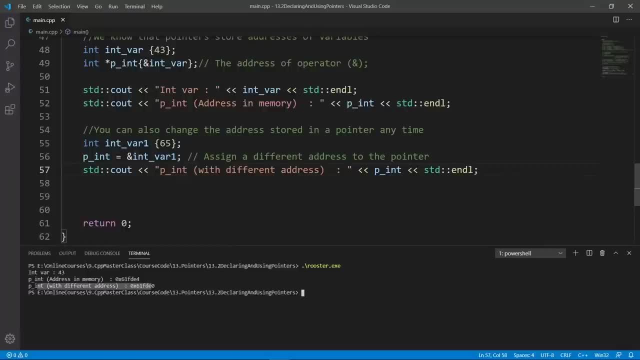 storing different things in our pointer. this is really cool. you can do something like this, and the next thing we want to see now is that we can't cross assign between pointers of different types, and what i mean here is that, for example, if we have two variables, 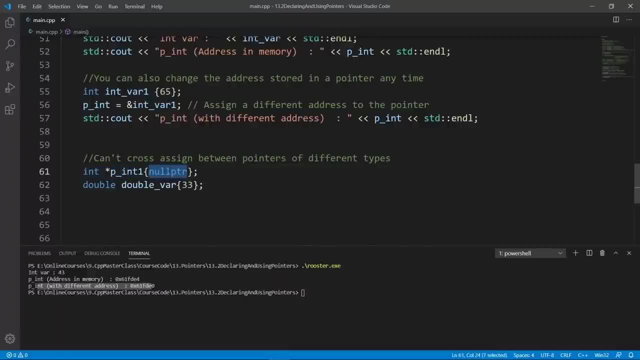 here. one is a pointer to int. it is initialized with no pointer and we have another variable which is a double var. it's going to be of type double and we can't do something like p, int equals address of double var. you can't do something like this. if you do it, you're going. 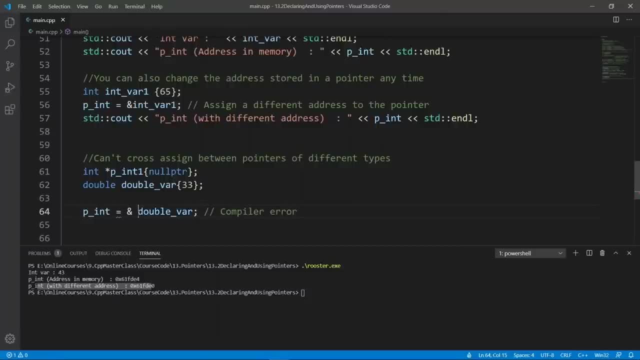 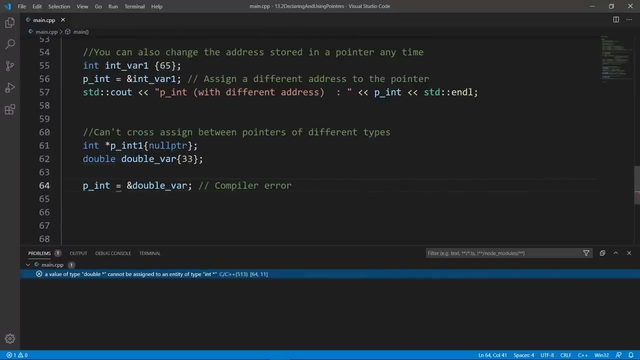 to get a compiler error and you see that we have squiggly lines in visual studio code. this is a good indication that something might be wrong. if we open the problems tab, we're going to say: value of double pointer cannot be assigned to an entity of type 8 pointer. so this is not something you 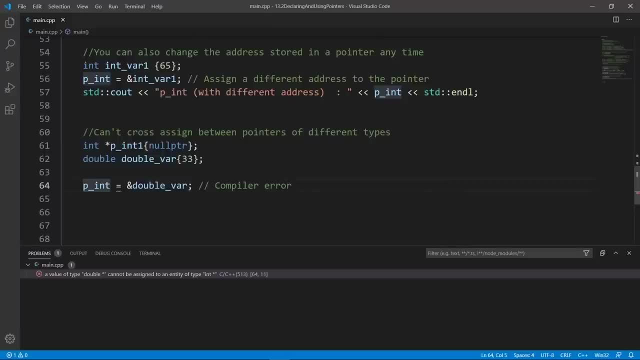 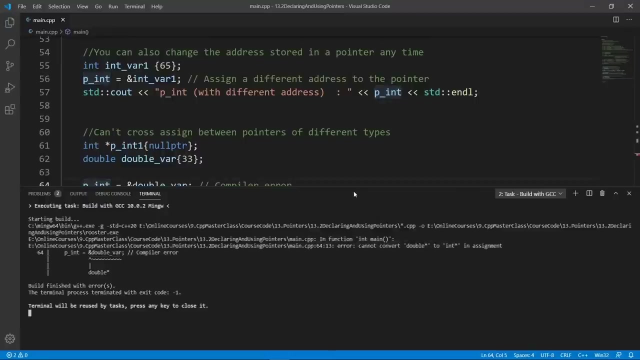 can do. if you do this, you're going to get a compiler error. be aware of this. visual studio code has warned us enough. but we can also try and get a clear compiler error by building this with gcc and we're going to get basically the same thing. you can't cross assign between pointers. 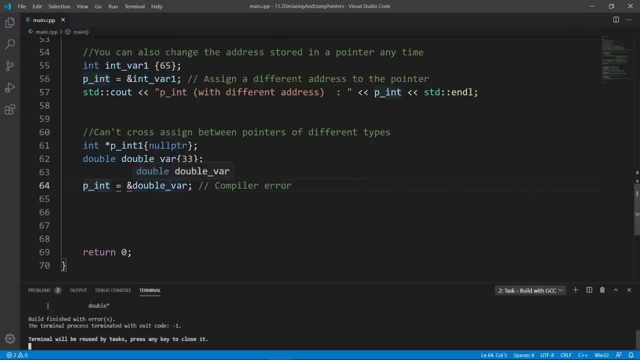 of different types. we are trying to assign a double pointer to an entity of type 8 pointer. we have to Gilman, that's a better answer, but if you're in gcc, first miss that example. I don't know you have to. if you do it in multiple loop changes, we're going to get theと思います. 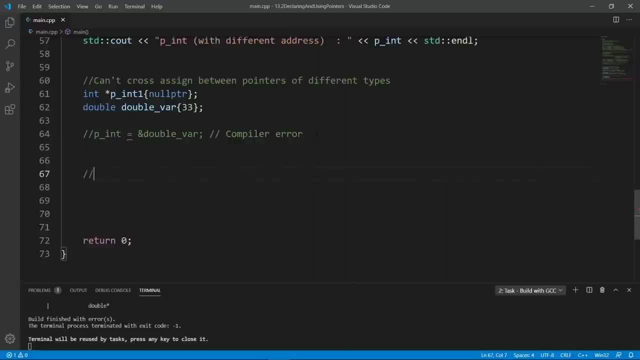 zię. ok, again, this is a simple오�разу. so there's some little次. 당신 grams, we put this in order. if have, for example, an int pointer, let's call it p and two, we have a variable like this. so let's say: 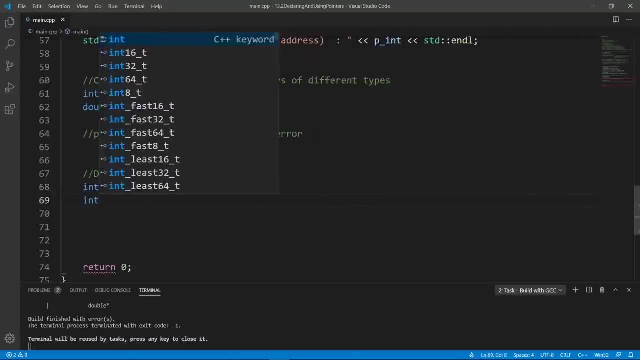 we initialize this with no pointer and we have an int variable and this is a 56, for example, and we do something like we do, say p and two, we're going to make it contain the address of each data. this is something you know you can do now. now we want to go through p into two to read: 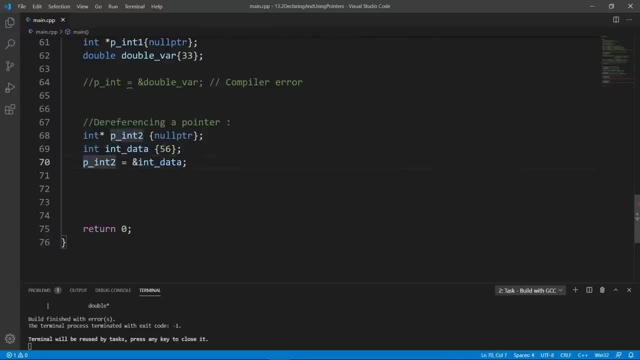 what is contained in int data, because p into 2 contains the address of our integer here. so what we can do, we can do stdc out and say value. and the syntax we use in c plus plus is like this: we say star and we say our pointer variable. we're going to say p into 2 and now if we run, we're going to 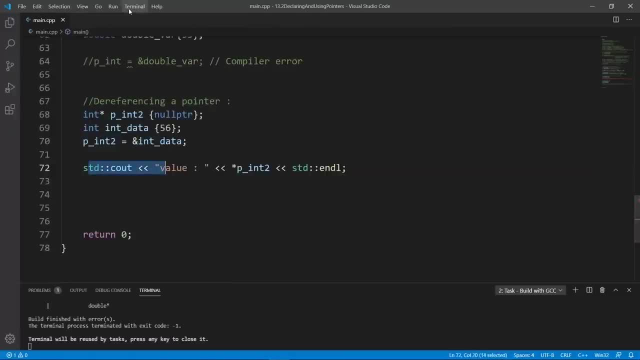 get the value here printed out. okay, now, if we try to build, we're going to build. fine, let's try with gcc. the world is good, we can clear so that the arrows from- uh, a previous run are cleared out. you see, the build is good, we can now run rooster and we're going to see that value is 56. we are successfully reading the. 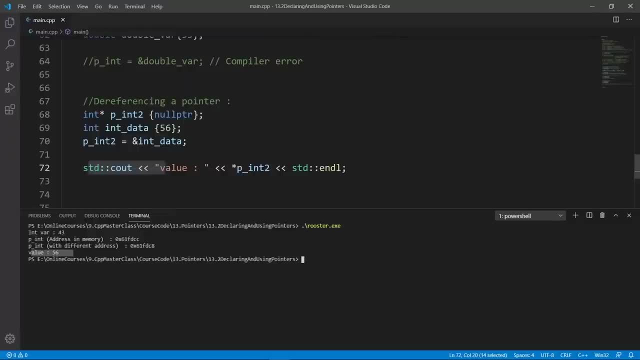 value stored in the address pointed to by our pointer. here, and this is the syntax used and this is court the reference in the pointer. we are basically reading something stored in the address of a pointer. this is what we're going to do: we're going to create a pointer here and we're going to 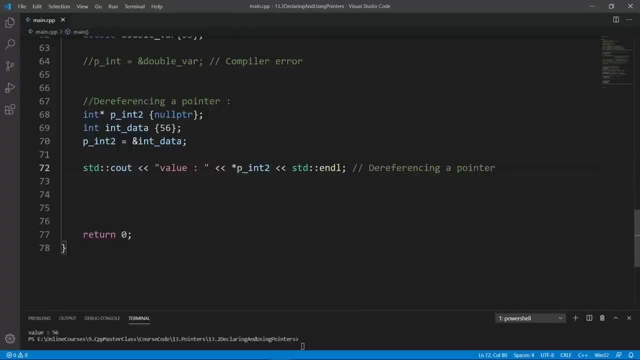 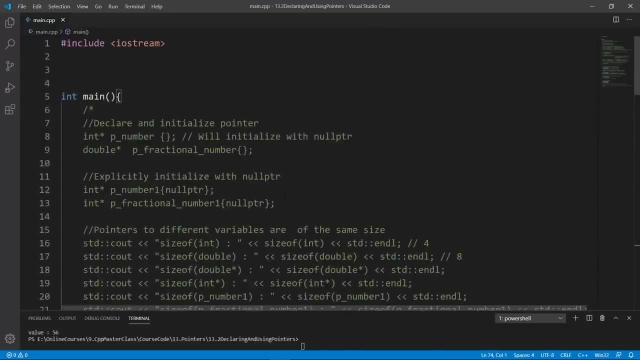 create a pointer here, and we're going to create a pointer here, and we're going to create a pointer, and this is really all we set out to do in this lecture. the lecture turned out to be lengthy, but we had a lot of ground to cover, and now i hope you have a good grasp on how to declare. 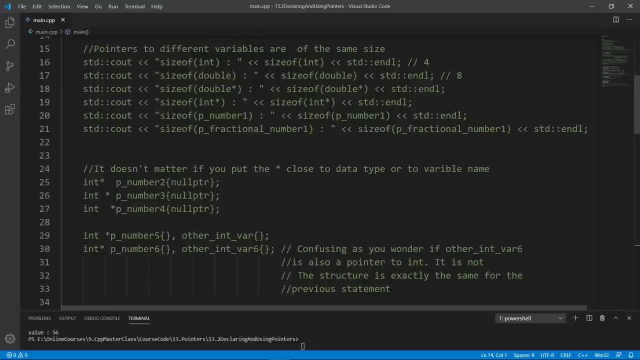 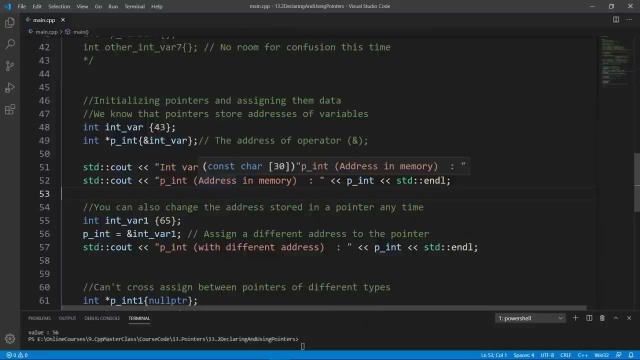 initialize and use your pointers to do all kinds of crazy things. we are going to stop here in this lecture. in the next one we're going to learn a little more about pointer to character types, because they are also special. go ahead and finish up here and meet me there. 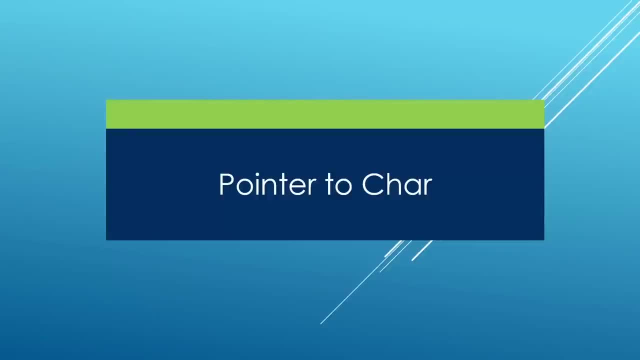 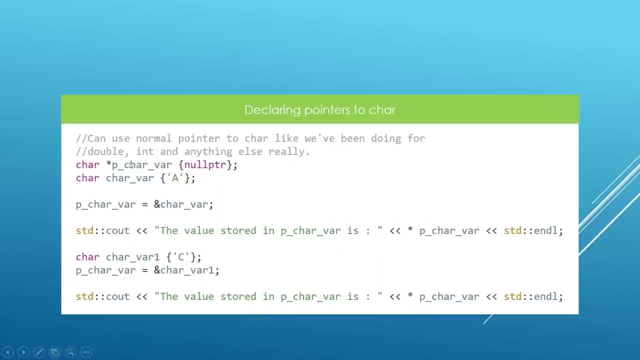 in this lecture we're going to explore pointer to characters and you can declare a pointer to a character just like this: we have car pointer and we say p car va recommend soldiers, so call it just like this. we have car pointer and we say p car var to give it a variable name, we initialize: 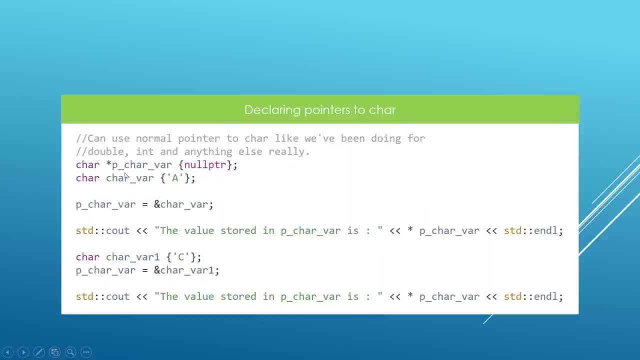 this with a null pointer, and after that we set up a character variable and it is called car var and we store in an a, an uppercase a. after that we take the address of car var and assign that to our commitment matrix, so that you' re the first to register that fracture, like anantom there. in order� Me. 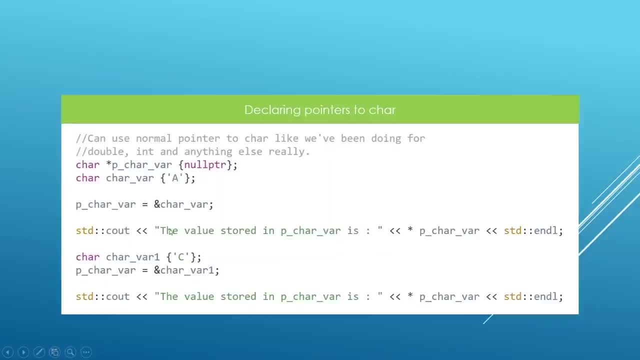 variable. this is how we store data in a pointer and we can go through this pointer to access data in this character variable. if we do something like this, we're going to print a down here, we declare another variable, we store in a c and we assign the address of this new character variable to our 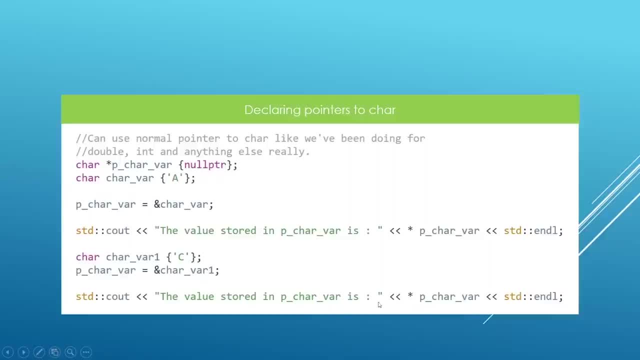 pointer variable and if we print this again we're going to get a c printed out. this is really what we have done in the last lecture. we are just extending that to character pointers. but with character pointers you can do something really special. what you can do, that is special. you can. 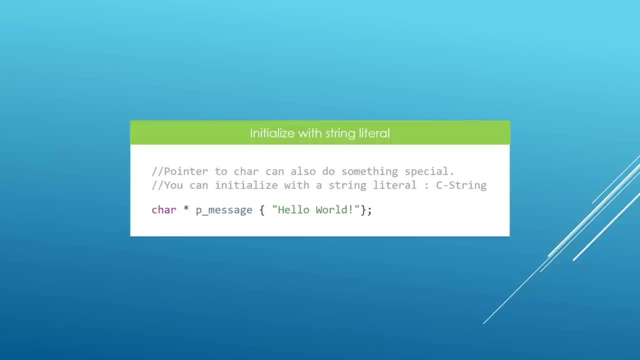 initialize that with a string, literal, something like hello world, which is wrapped in quotes like this: when you do something like this, the string here is going to be expanded into a character array and the first character of our array is going to be pointed to by p message here. 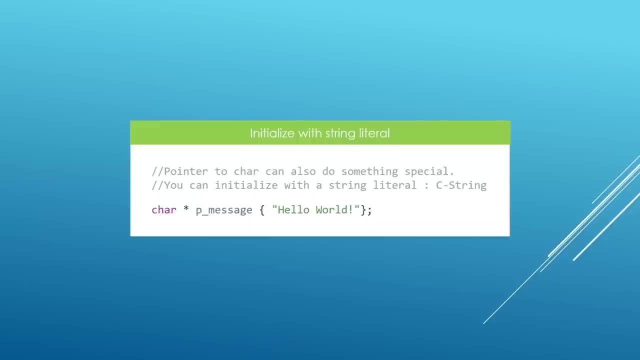 this is what we mean. i realize i might be throwing a lot of things at you right now. i am mixing up arrays and pointers, but they have a really strong relationship and we're going to learn about that in detail in a few lectures ahead, but for now, think of it like this: this hello world. 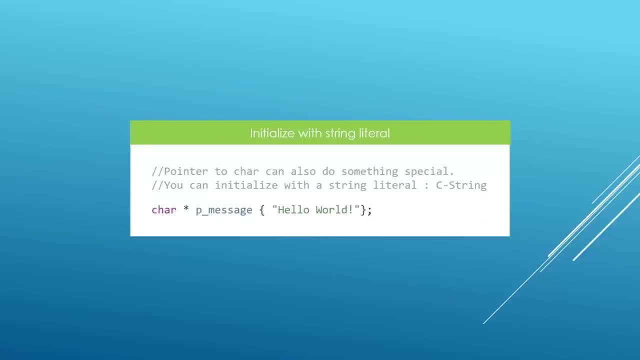 string is going to be turned into a character array and the p message is going to point to the first character in this array. here, this is what is going to happen, and this is going to give us the ability of treating our strings as character pointers, and this is going to come in handy at 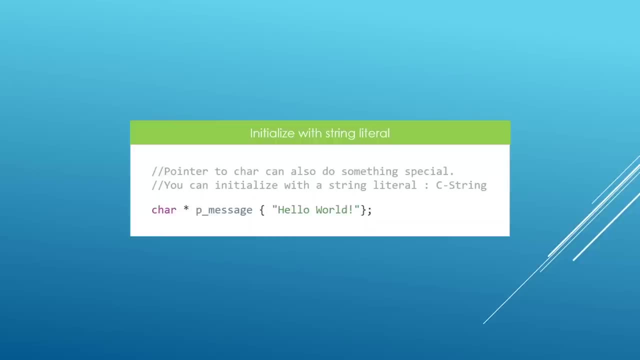 many occasions. one thing i should tell you, though, is that some compilers will refuse to compile this code. for example, visual studio 19 that i have installed on my computer right now, is going to refuse to compile this code, and the reason is the compiler is going to expand this string into. 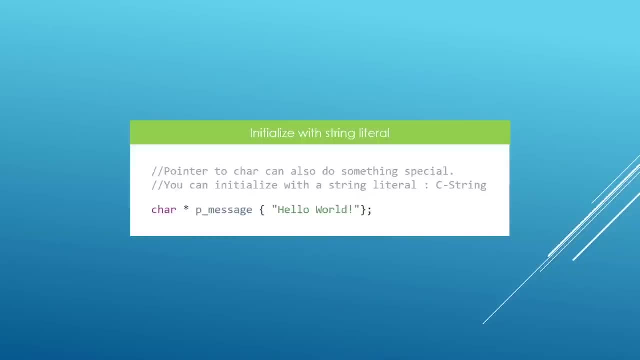 a character array of const car, and here what we are using to point to that is not the cost car pointer. so this pointer here can be used to try and modify data into an array of const cars and that's going to be disastrous because if you try to modify that that's going to fail and that's. 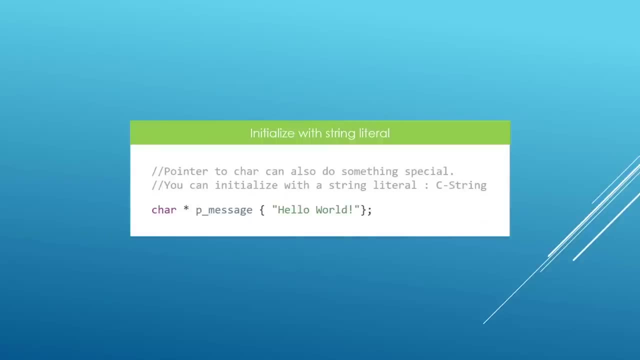 not going to be good. so some compilers are going to try and protect you from this and force you to use pointers that are qualified with cost to really mean that they are caused to pointers and to get the code to work. we will have to do that and i will show you how we do that in. 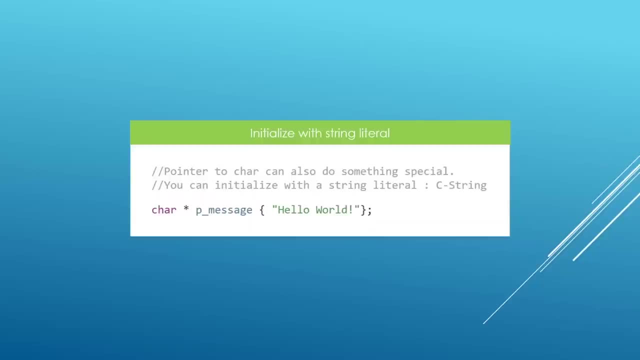 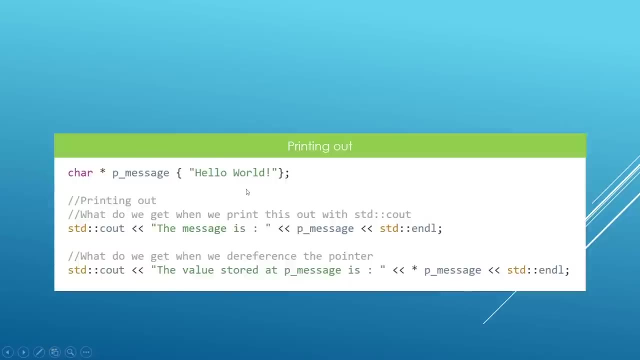 visual studio code, but i had to tell you this in case you just want to jump ahead and try this code out. if you get a compiler error, that's going to be the reason. now that we have our string stored in memory, we can really print it out like this: if you print p message, you're going to get the string. 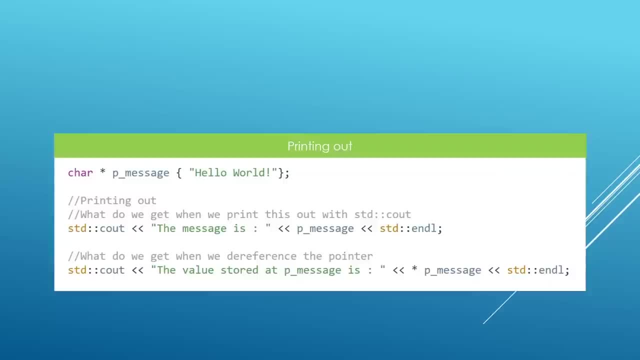 printed out. but i want to give you a question here. what do you think we will get if we dereference p message? try to think about this. i told you that the compiler is going to expand this hello word string into an array of characters or, to be specific, an array of const cars and p message. 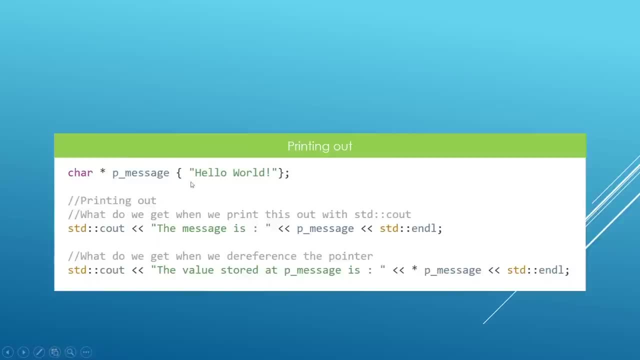 is going to be pointing to the first character in that array. so if we dereference p message, we're going to get that character printed out. in this case we will get an h, and that's what is going to happen here. but character pointers are special in that if you print them out, directory, the compiler is going to do its magic. 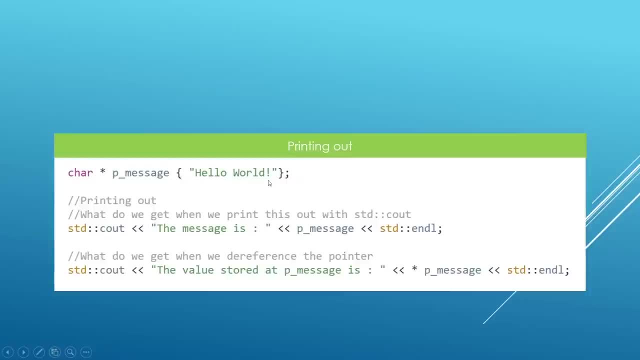 and make it possible to print out the entire string that is stored in p message here. that's how character pointers are special and you really need to be aware of this because this is going to come in handy many times. just to emphasize that this is going to be expanded into an array. 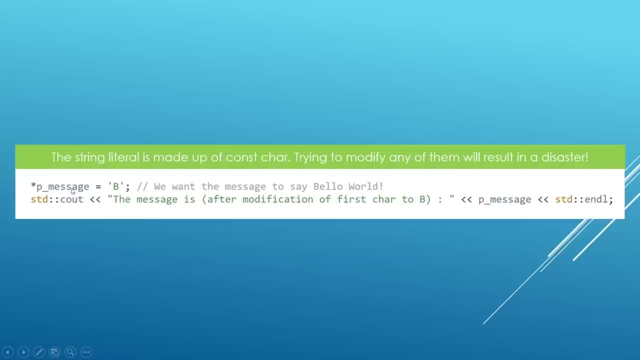 of constant characters. if we try to modify something inside p message here, for example, we try to change the h into a, b- we can try to do that because p message is pointing to the first character. so we can try to dereference and assign a new value. and if we do that we're going to get a compiler error or even 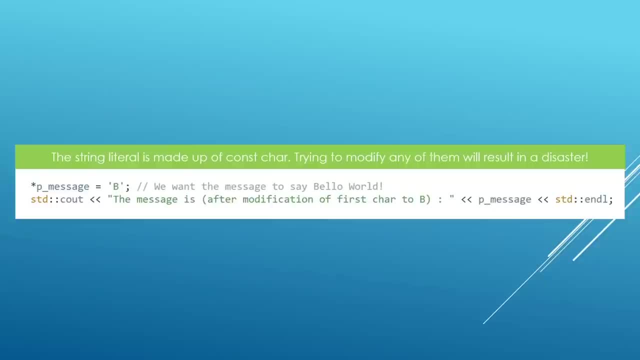 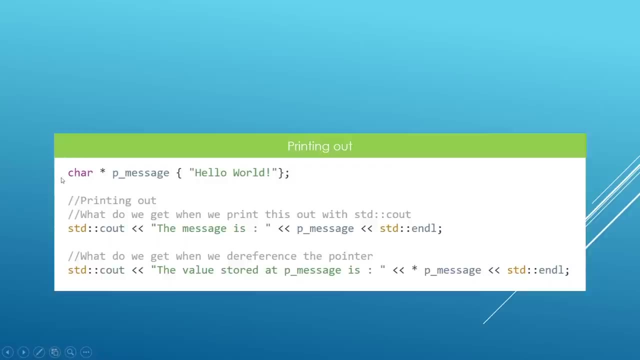 worse, we might get a crash at runtime. so this is something you shouldn't really do and you should really flag your p message here as the cost car pointer, and that's going to prevent you from doing things like this, which may turn out to be very bad, but most compilers are going to even prevent. 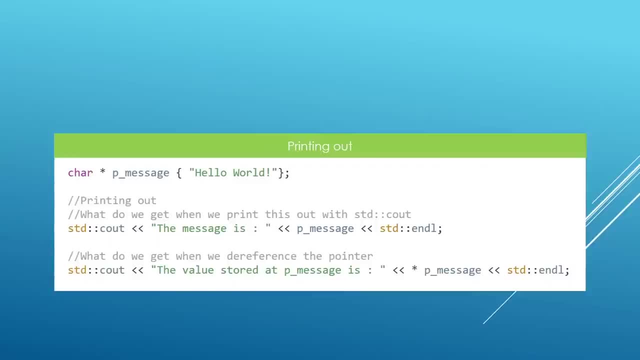 you from compiling this thing in modern times. for example, if you are using a very recent version of visual studio, you're going to get a compiler error. but i don't believe gcc is going to give us a compiler error, so we will have to try this out and see how it behaves, but the message is: 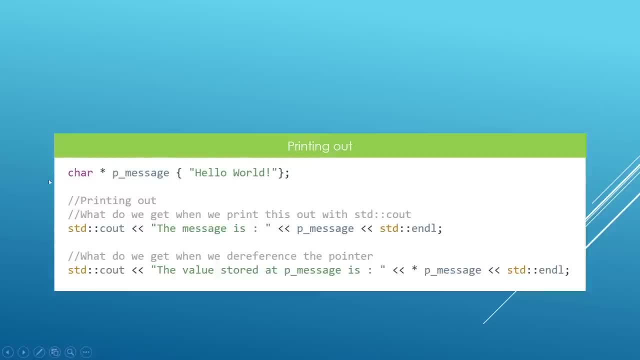 if you have to do something like this, make sure you use the cost car pointer, and you're going to be playing on the safe side. okay, now i think you know enough about character pointers. what if we want our users to be able to change this string and make it be? 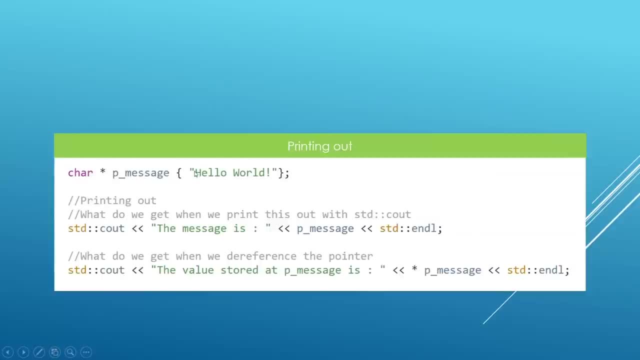 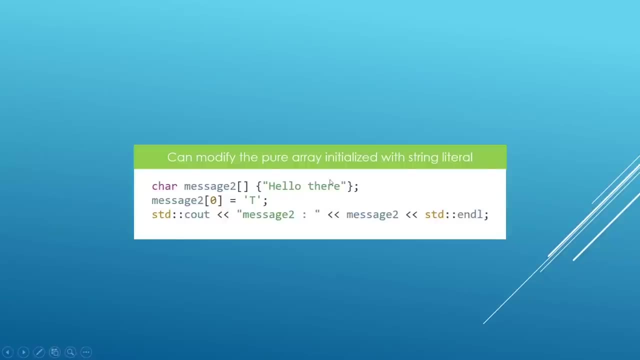 something else. for example, change the first character here into a, b. well, in that case, don't use character pointers. use regular arrays, like we have seen before, so you can set up an array like this. it's going to be a character array and you can initialize it. 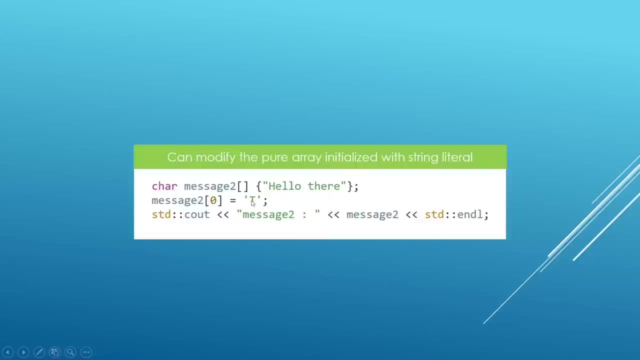 with a string- literal, and this is going to allow you to modify things inside. so if we do something like this, we will get the message printed out and the message is going to be tello, because we changed the age to be a t, and this is going to work. so this is something you really need to be aware of. 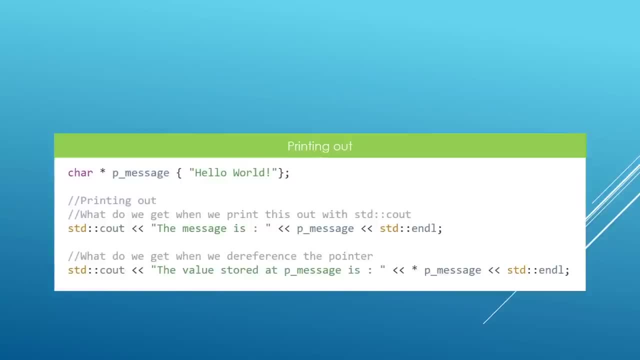 but character pointers are very helpful in many cases, and in most cases you just want to store the string and print it out. you're not interested in changing it. so that's why this is going to kind of come in handy in a lot of occasions. now that you know this, we're going to head over to visual. 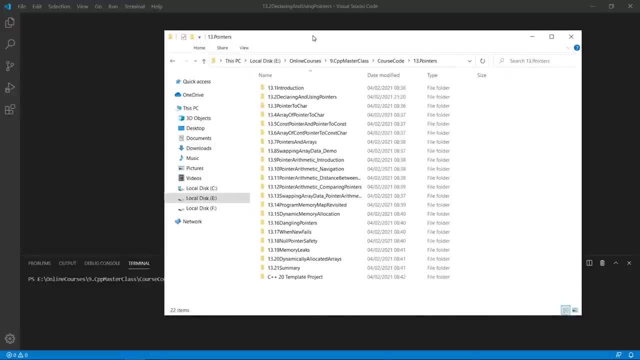 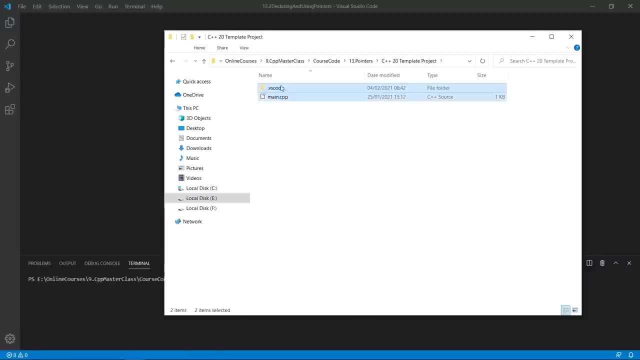 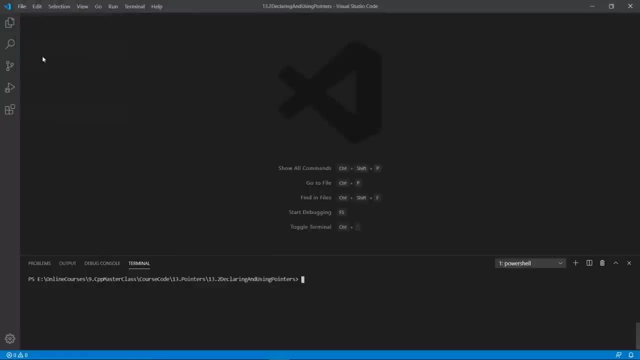 studio code and actually try this out. okay, here we are in our working folder. the current project is pointer to car. that's what we are exploring here. so we're going to grab our template files and put them in place and we are going to open this thing into visual studio code. 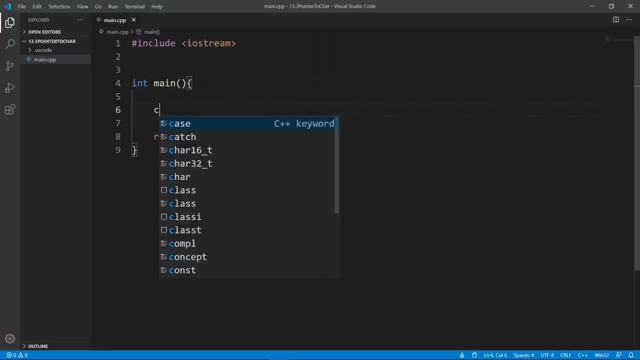 and we're going to jump into here and set up our first const car pointer. let's do car pointer to see how this thing behaves. we're going to call this message and we're going to initialize this with our trusty message here: hello world, okay, once you do something like this, your string is: 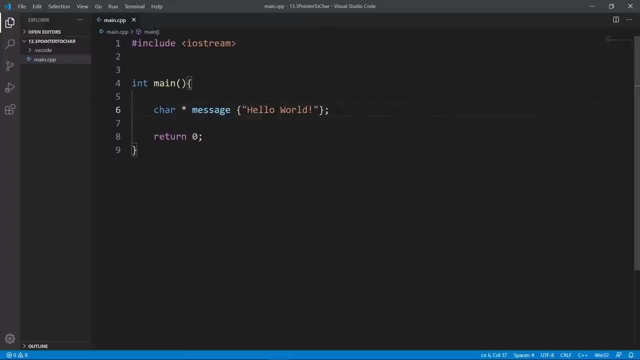 going to be referred to by message. let's try and compile this and see that gcc is happy. we can compile with gcc and it's going to tell us we can't really do that. and this is really good for bits converting a string to constant car pointer. so what we are doing 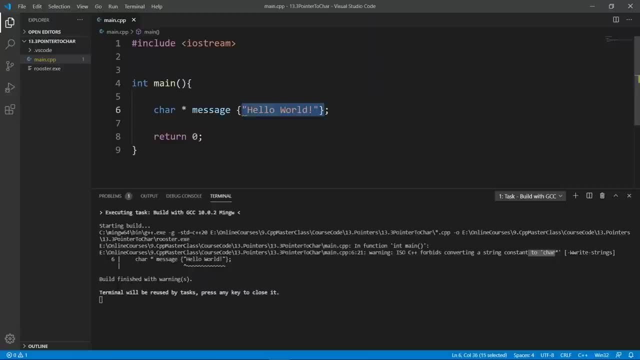 really is making an array of const characters and refer to it as a car pointer, and this is not going to work. this is a good thing. so you can't really do this, and this is a good thing, and let's try and see if visual studio can actually do this. we're going to build with msvc. 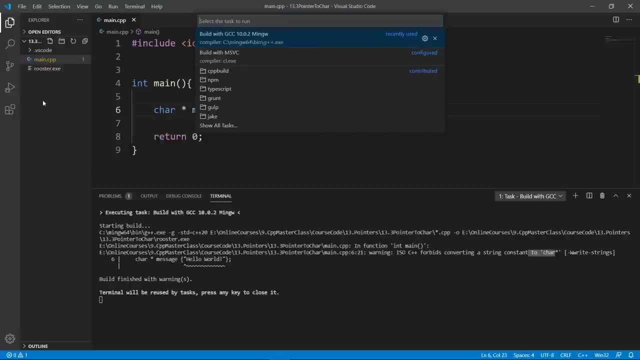 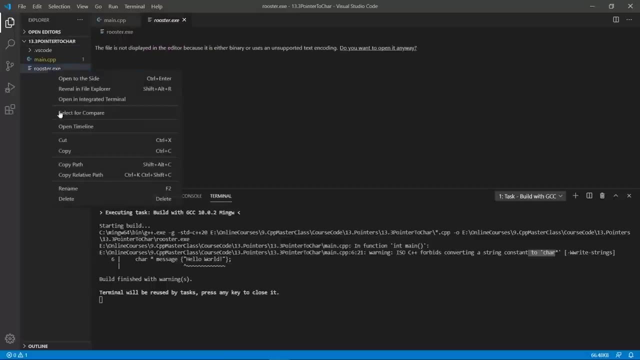 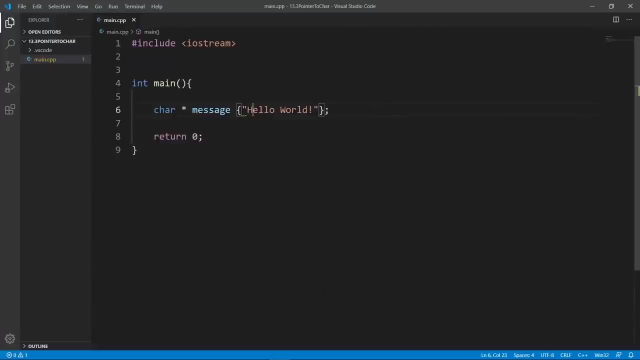 in this case, let's do read to booster. before we do that, we can right click to it and say delete. let's click to it first, make sure it is selected and hit delete to remove it. move to recycle bin, in this case. now we're going to clear here. let's bring up our terminal again and we're going to clear. 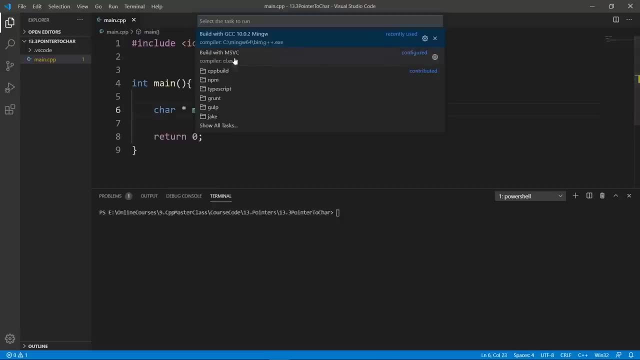 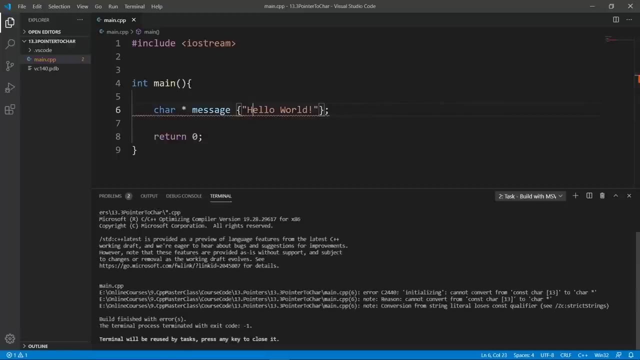 and we're going to build with gcc, but you're going to choose the msvc compiler. if you're trying to build this uh world, finish it with arrows and the error is going to be basically the same thing. this line here won't work. what we can do is make this cost and make. 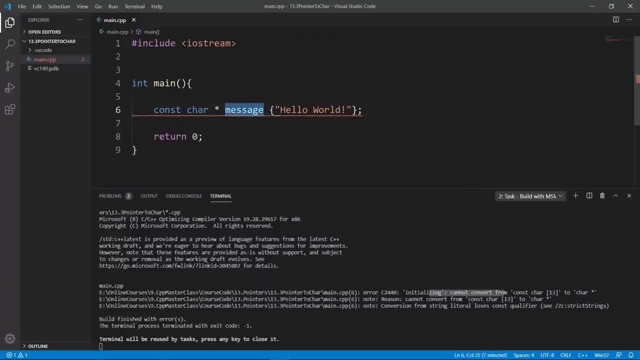 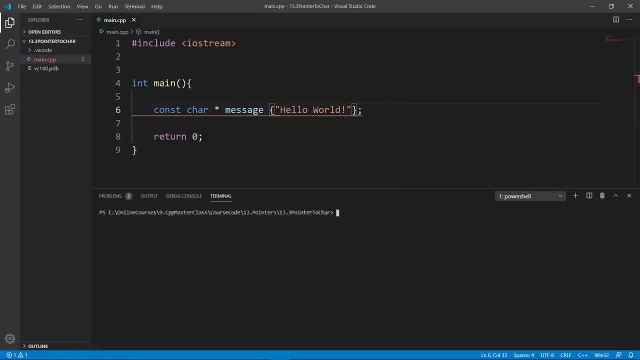 it super clear that message here is going to point to an array of const core if we try to build again. i think we're going to be good now, so let's try and do that. we're going to build with msvc this time and world finished successfully. now this is really cool and we can print this out. we. 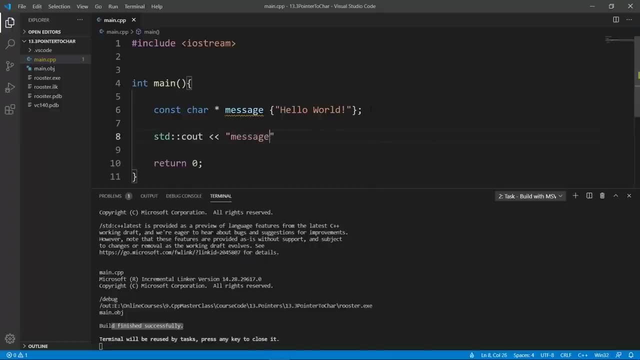 can say sdc out and we can print this out, and we can print this out, and we can print this out and message, and we're going to say message and this is going to work. let's go back to gcc, because that's my favorite compiler and you see, 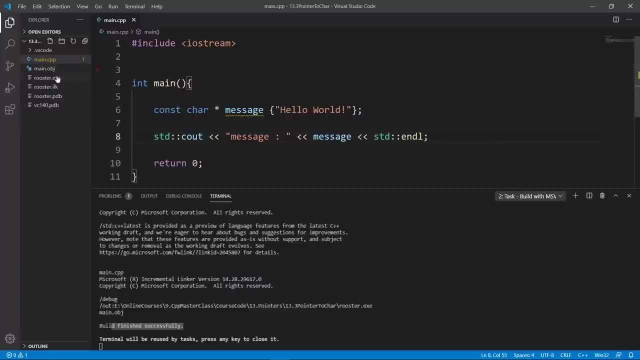 that the compiler from visual studio is going to clutter our folder here with a lot of files. we don't want that. what i'm going to do? i'm going to select all this clutter here and remove that, and i'm going to hit delete with the right click and it's going to go away. we're going to go back. 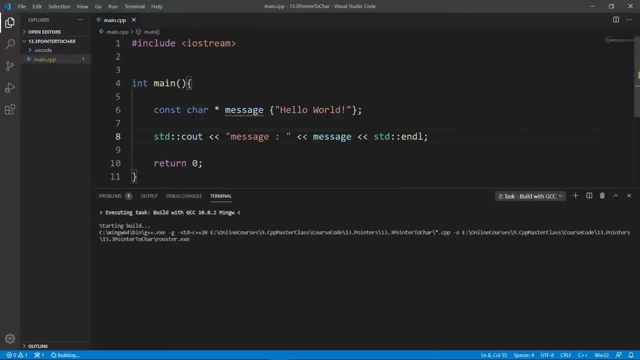 to gcc and use it and build with gcc. the build is going to go through because we qualified our character pointer with cost here and everything is going to be good. be sure you know what is happening here, because this kind of problems can be really hard to solve. okay, now that we have this, we can 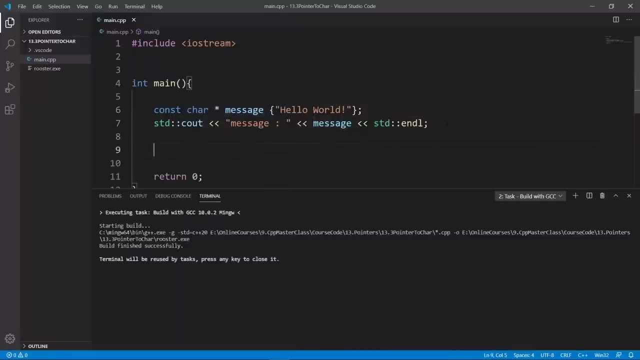 try and change something inside, but the compiler is not going to allow it. so if we try and do something like this is not going to work because maybe we're going to have to do something else. so message is a pointer to cost core and we can't go through this pointer to modify something. 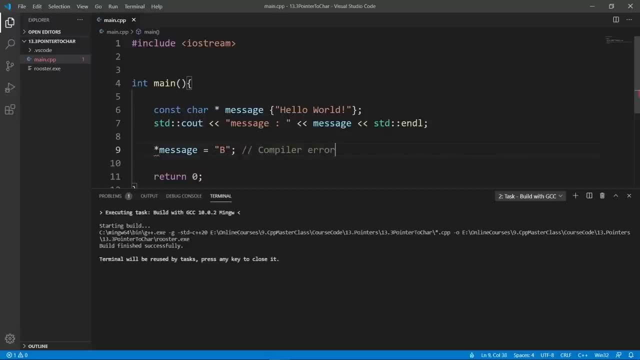 so we're going to get a compiler error. this is something you should know. but we can add the reference, this pointer, and print something that is inside, and i want you to guess again and see that you can come up with what is going to be printed if we the reference. 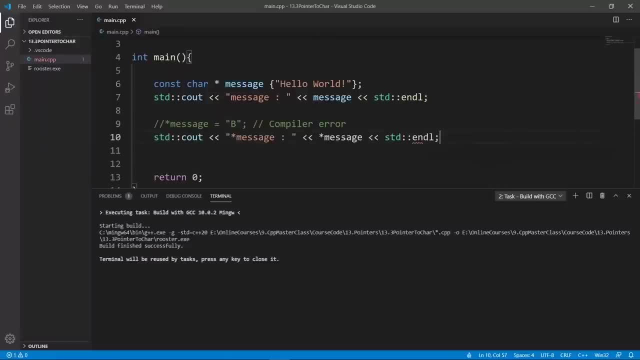 message and print out when we run this program. if we have this thing printed out, here again we are referencing the pointer and printing whatever result we get from that. remember that this string literal is going to be turned into an array of cost cars and the first element of that array. 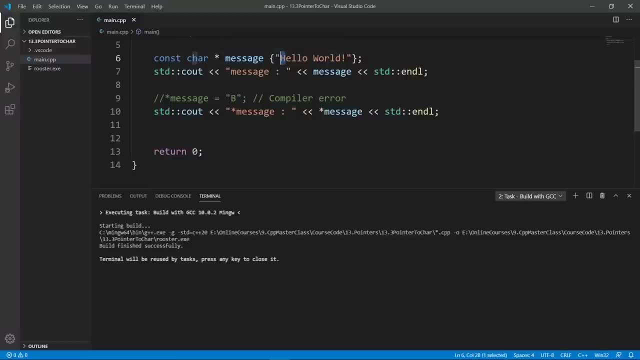 is going to be pointed to by this message. car pointer here. so if we dereference this thing, we should get the h here printed out. that's what i think we should get. let's try and build with gcc. of course the world is going to be good. let's clear and run rooster. see that message. 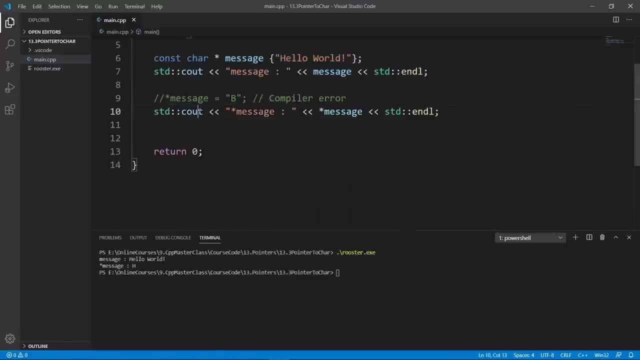 is h. this is exactly what we expect here. now that we have this working, what if we really want this thing here to work? what if we wanted to allow our users to go through this message thing and modify what is stored inside, because sometimes that's going to be useful? okay, we want to allow. 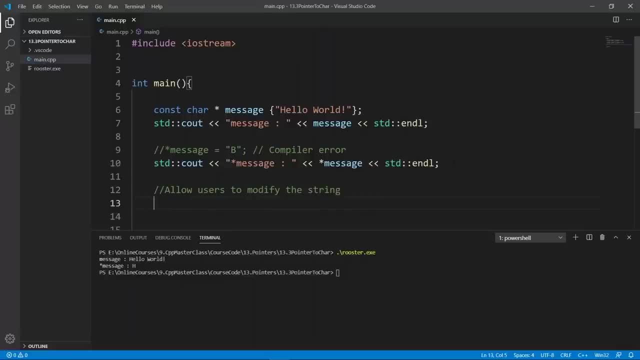 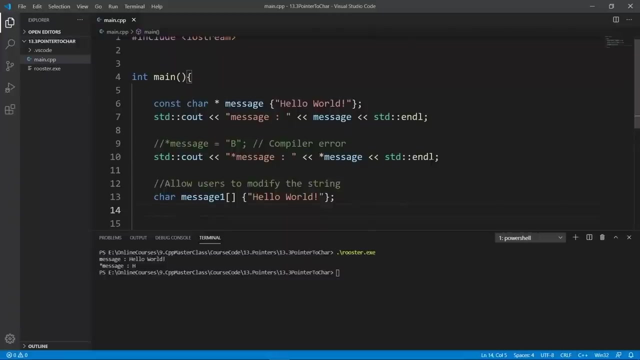 our users to modify this string. if you want to do that, you can use row character arrays and the way we do that. we can say car message one and we can make it an array and initialize that with hello world. and once we do this, we can go through the angle bracket syntax and modify the first character or whatever. 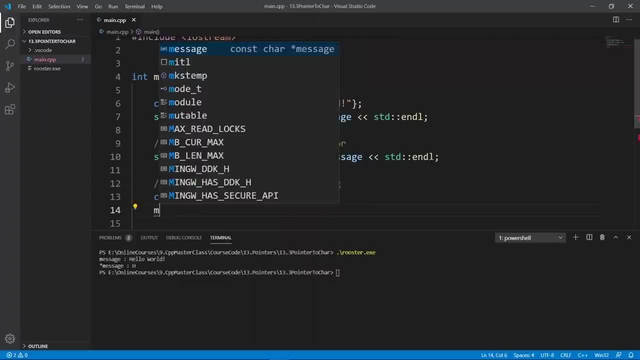 character we really want to modify in this string here. in this case we are going to target the first, so we're going to say message one and we're going to grab the index zero, because that's going to be the first character here, and we're going to assign a new character, let's say b, like we just said, and 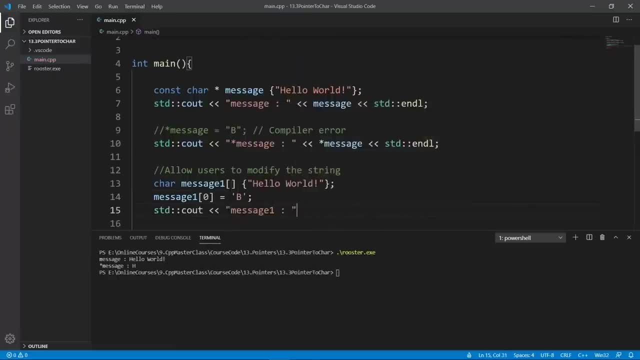 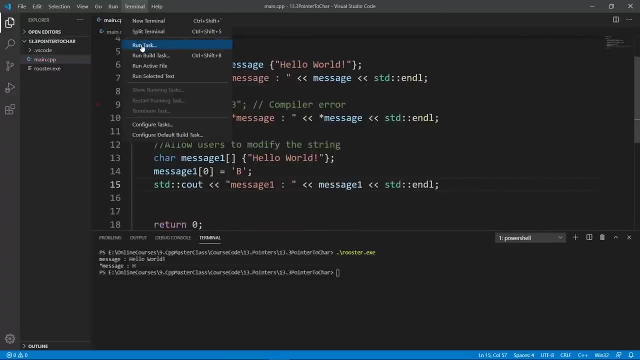 if we print this out, say message one and put that out, we're going to see what comes out. if we run this program, we're going to world with gcc, so let's do that. the world is good, so we're good here. and if we run, we're going to get below printed down and we have successfully changed this thing here. 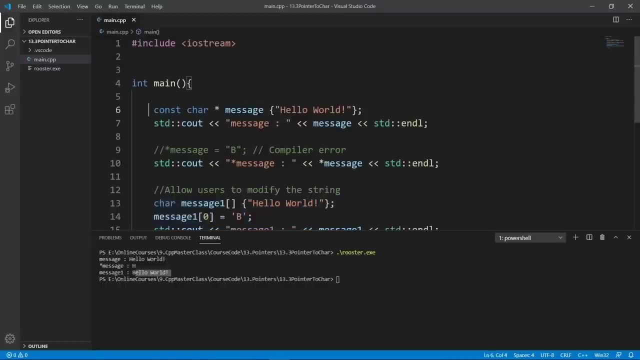 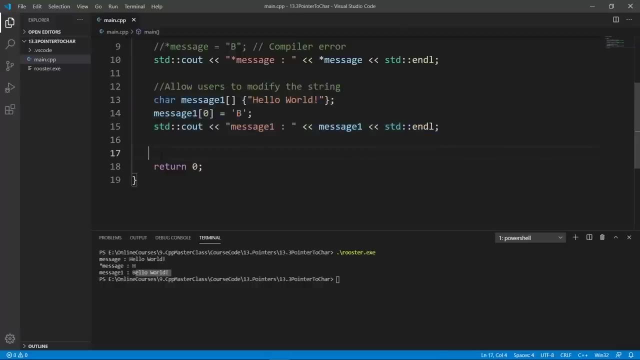 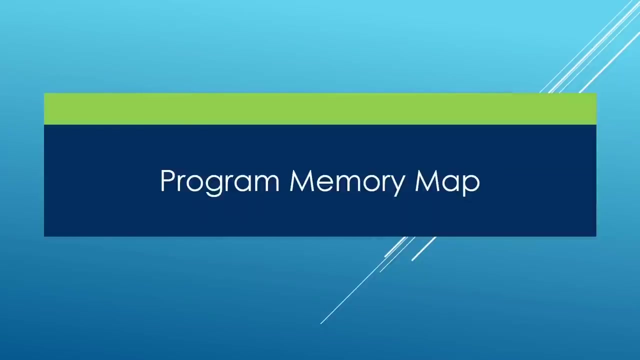 so if you don't want to allow modifications to your strength, use this thing here. if you want to allow modification to your strength, use this syntax here. and this is really all we had to say in this lecture. in this lecture, we're going to revisit our idea of a c plus plus program. 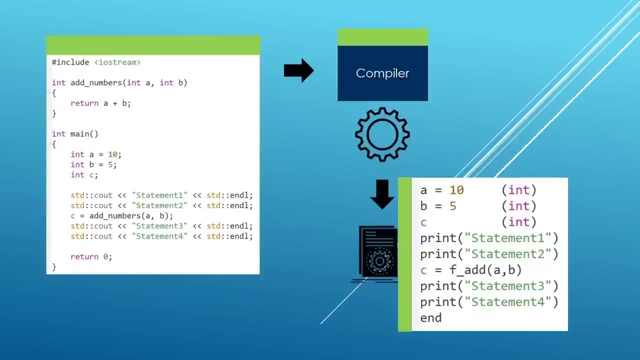 memory map. we have seen that the c plus plus development workflow really goes like this: we have a program typed out in our ide, we pass that through the compiler and we get a binary executable which is a binary representation of the code we have in our c plus plus program. 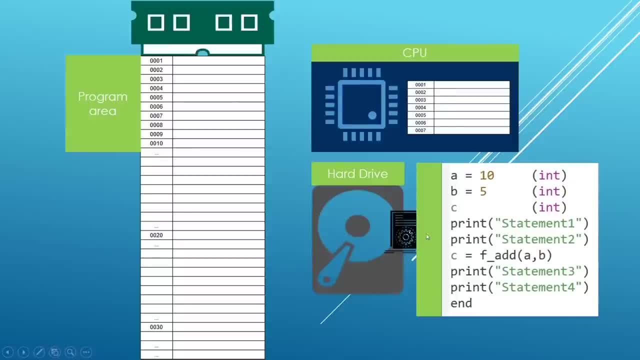 you can then run that program on an operating system, for example here i am on windows. if i double click on my dot exe file, for example, our applications are called roosterexe. you've seen me run this a thousand times by now. if we double click, this program is. 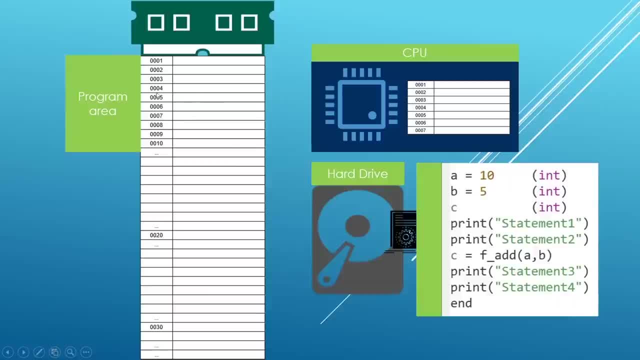 going to be loaded in our computer memory, and by memory i mean random access memory. the memory that is going to be actively running things when they happen in your computer is different from the hard drive storage. that can also be called memory, and this can throw off a lot of beginners. we are 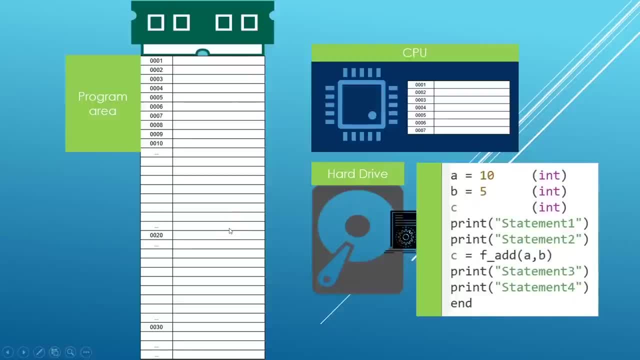 talking about ram here, when we mean memory, random access memory memory. to be exact, if you double click on your program or open it on the terminal, like we've been doing, the program is going to be loaded in memory and it's going to be stored in a special 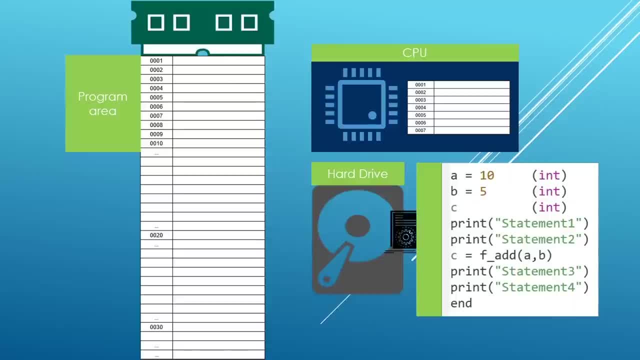 section of memory called program area, and so far we have been thinking that our program is really loaded in real memory on our computer. but that's not the case. it is an idea of the memory that the program thinks it has, but it's not the real thing. 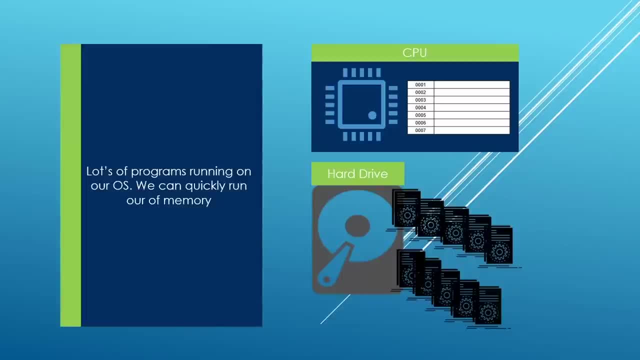 and i am going to explain. but before we explain, let me elaborate on the reason why this is done. if we have many programs and each program is going to use real memory on our computer, we could quickly run out of memory because there are many programs. you might even have. 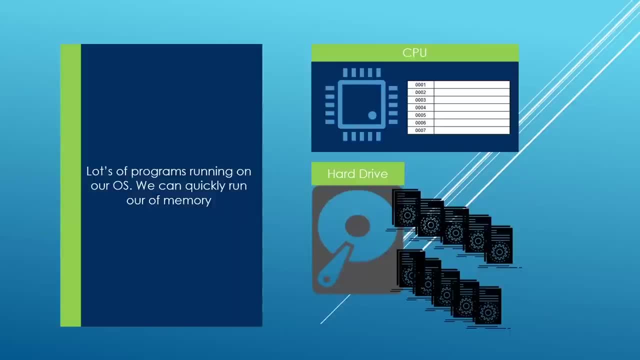 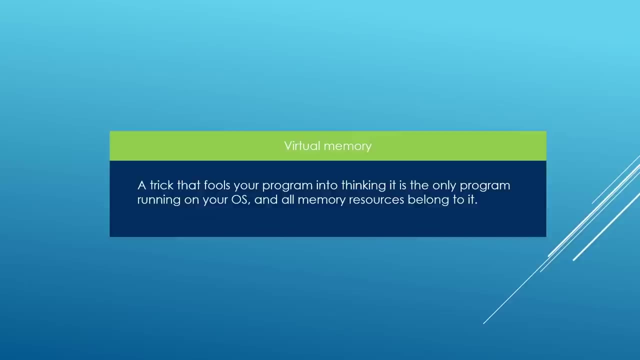 hundreds or thousands of programs running on your computer. you may never have enough memory to run them all if real memory was used by each program. so the idea was born to create what is called virtual memory, and it is a trick that fools your program into thinking it is the only program. 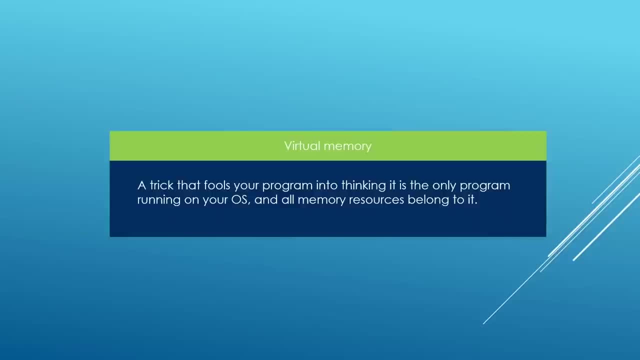 running on your operating systems and it owns or the address space or all the memory on your computer. that's what your program thinks and the view that your program has of that memory is called a memory map. each program is abstracted into what we call a process- you can think of roosterexe that. 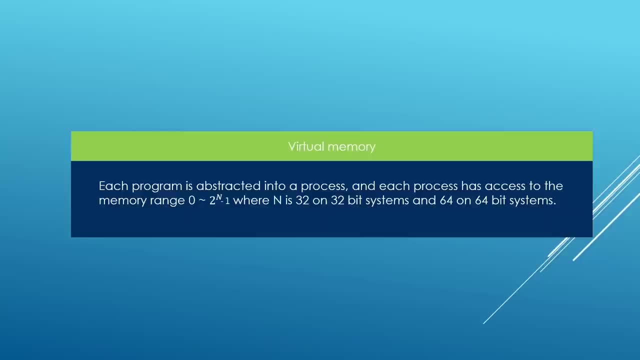 as a process on the system, and each process has access to the memory range between 0 and 2 to the power of n, where n is the number of bits that your operating system supports. for example, i am on a 64 bit operating system, so the range for my memory is going to be between 0 and 2 to the power of 64. 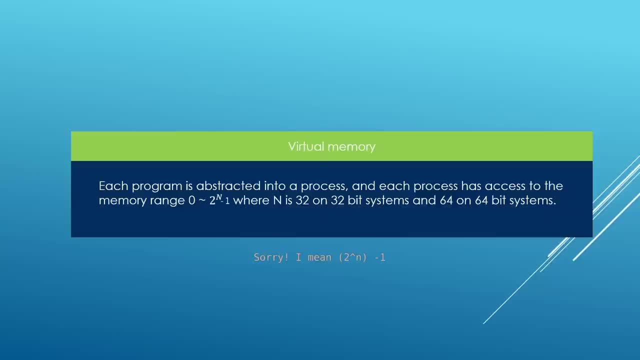 and that's a lot of memory. my program is going to think that it owns all that all and it can never do whatever it wants. if you are on a 32-bit system, that's going to be between 0 and 2 to the power of. 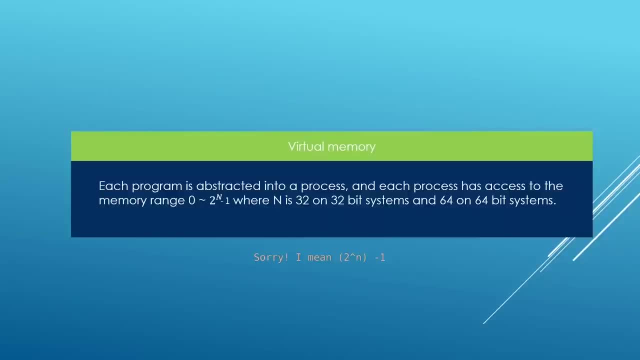 32, and that's going to be your virtual memory, the amount of memory that your program thinks that it owns, and it happens to be the entirety of your ram that you have on your system. each program basically thinks that it owns the entire memory and it can do whatever it wants. okay, so we have 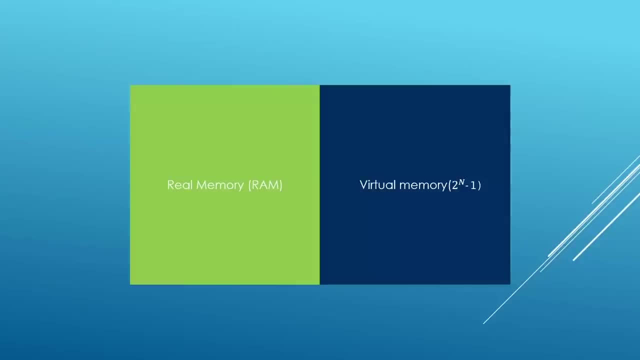 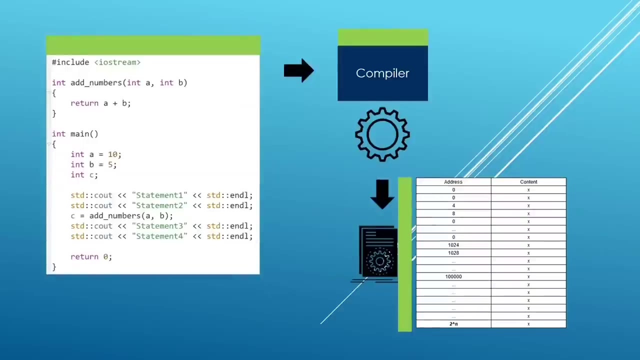 the real memory, which is random access memory, and we have virtual memory, which is going to be between 0 and 2 to the power of n. okay, so now we're going to update on the idea of the program execution model, because now we know more, we know about virtual memory. 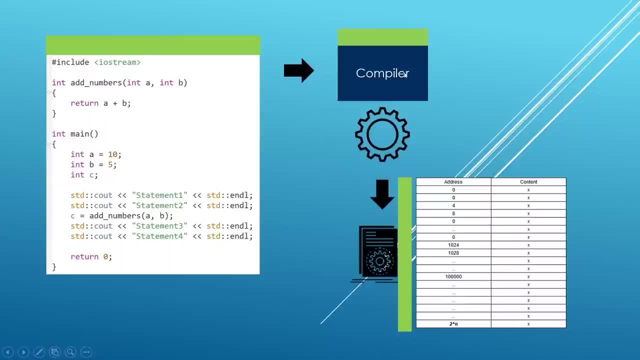 here is our c plus plus program. it's going to go through the compiler and we are going to generate a binary file which is going to be a representation of how things are going to be laid out in memory in our program and if we run the program it is going to go through the program and it is going to go. 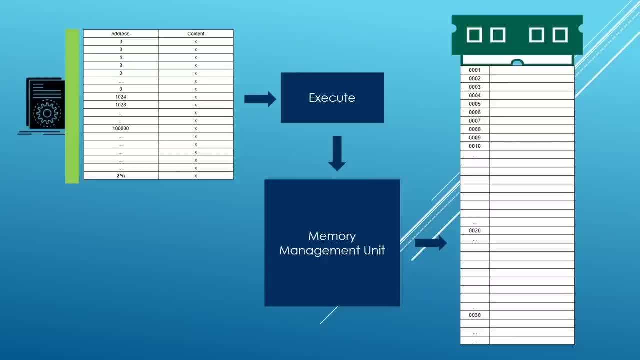 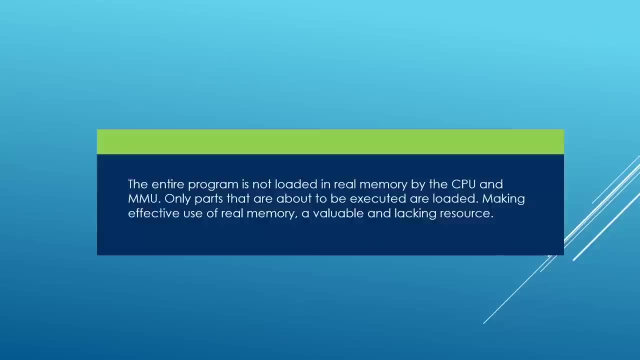 to a section of the cpu called memory management unit, or mmu for short, so that mmu is going to be basically transforming between the memory map of each process and the real memory layout that we have in ram. what the memory management unit does is really transform between the representation we 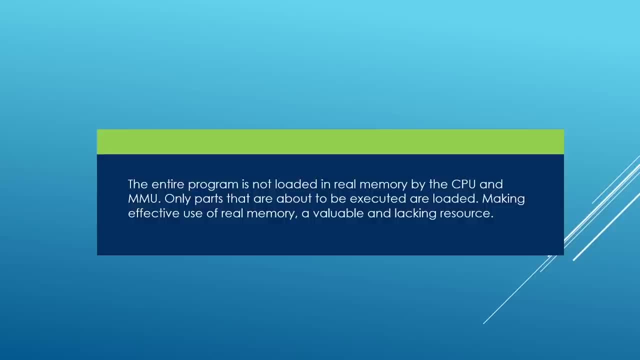 have in the memory map and the real thing we have in ram. the entire program is not loaded in real memory by the cpu. only parts of the program that are really going to be used soon are loaded in memory, and this is going to make effective use of the memory. parts that are not likely to be used are 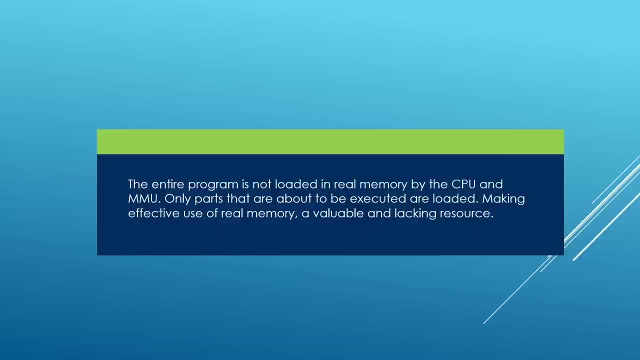 going to be discarded from memory and stored on the hard drive instead, and this is really cool. please note that the real way these things are done is really complicated, but it is buried down into the logic of the cpu and whatever. you don't really need to worry about this as a c plus plus. 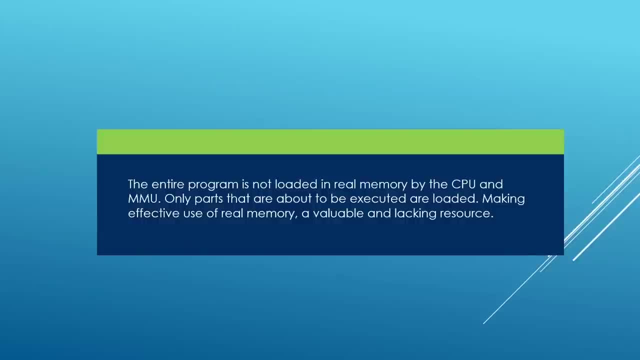 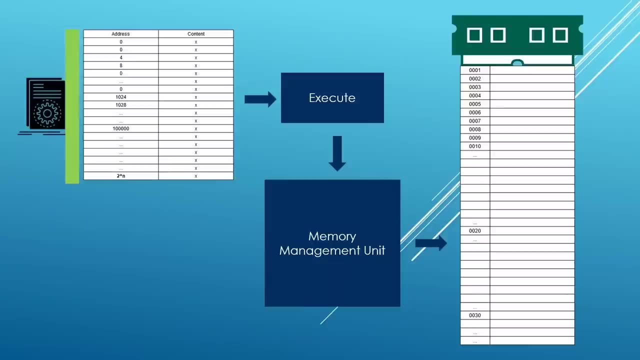 but there are a few things you need to know, as we are about to see in this lecture. so memory management unit helps out in mapping between the memory map you have in your program- basically the idea that your program has of memory, and the real thing that we have in memory. okay, here is a slide. 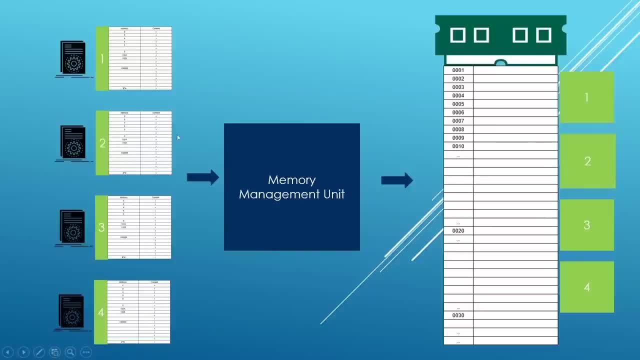 that is going to drive this home. we have a few programs with their own separate memory maps. we have program one through four. if we execute them, the system will start entering memory. I'd like to make a screen. read it out so you can see it. if I click on it and there are only two programs on it. here we have one program that is read out using the investors. the first program is the memory map and the second program is using the cpu. that is called memory map. so basically any program that is added will be visible to us and if you hit that here on this slide, you will see the cpu you have. here is the cpu that is. 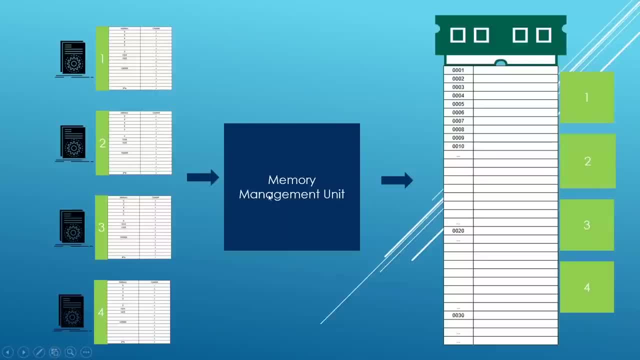 we execute them, they are going to go through the memory management unit and the memory management unit is going to assign them sections on the real ram that we have in our computer and they are going to be using that section on the real random access memory that we have on our computer, the. 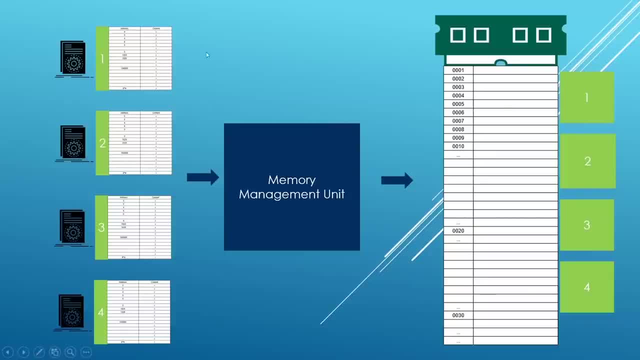 thing is your program is going to really think it owns the entire thing, but it's not just going to be using a part of it and the memory management unit is going to be transforming between the idea that your program has and the real memory that we have on our computer and the memory map. 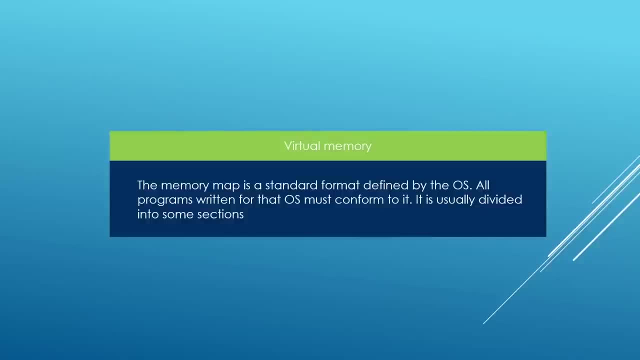 is a standard format that is defined by the operating system. this is why, for example, you can't take an executable that was set up on windows and directly run it on linux. this is an operating system thing. the memory map or the structure of your program is defined by. 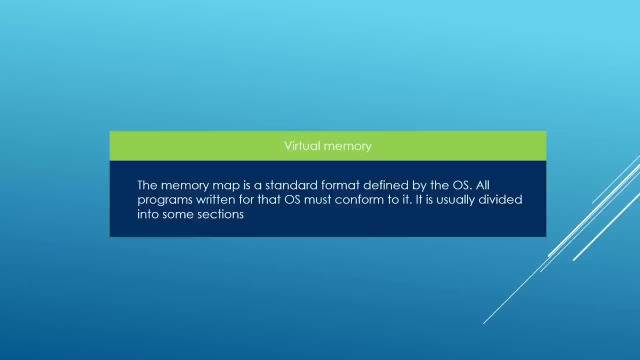 8.3.1.. henry and x, element 0.3.2.. We know how complex this process is, but i'm not going to yummy the operating system that is going to be running that program. so all program returns for an operating system must conform to the memory map, that is. 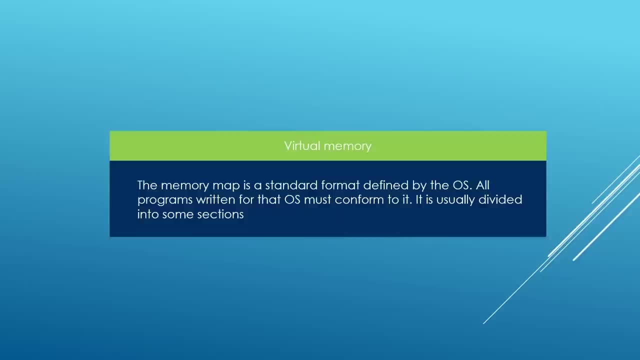 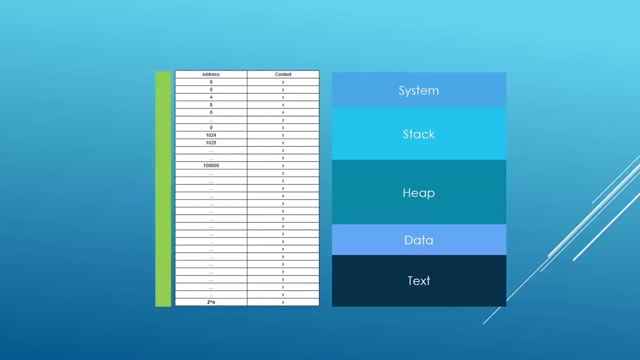 defined by that operating system, so all programs on Windows. if you had a way to go in and look at the memory map, they are going to be pretty similar. so we have been talking about the memory map, but what does it look like? well, here is a slide that is going to try and clear that out. so we're going to have a bunch. 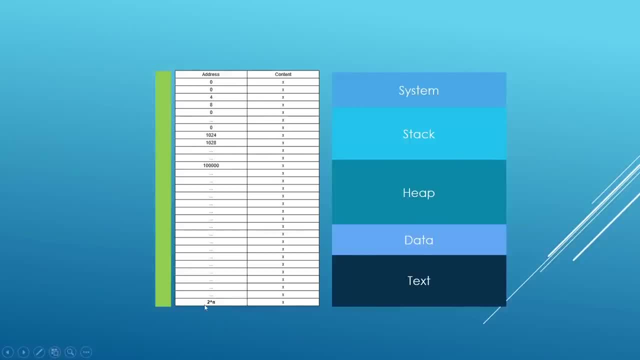 of memory locations, from 0 all the way to 2, to the power of M, and the memory map is really divided into a lot of parts. for example, we have the text section, we have the data section, we have the heap stack and system, and this is. 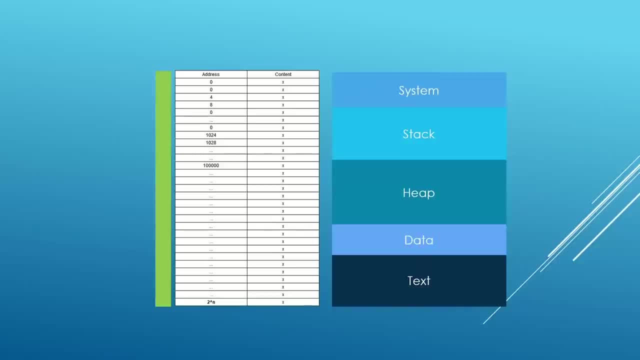 one view you can have on this. there are a few different versions of this slide that you're going to see on the internet, but what is really important is stack and heap. for our purposes here, stack is what is going to store our local variables. thank the a that we have. 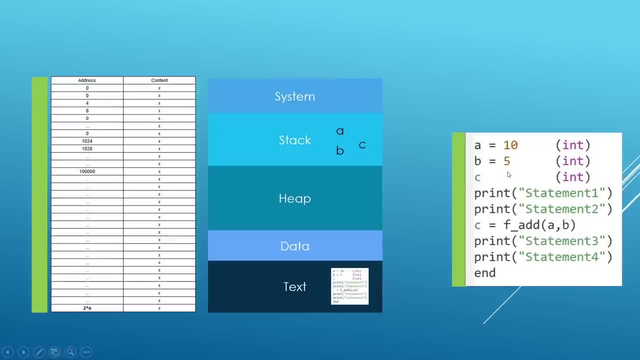 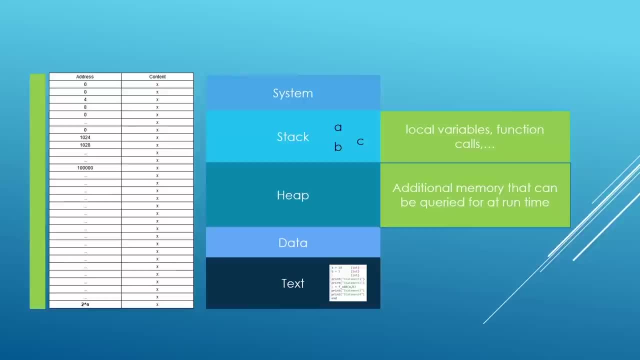 here in main. BC thanks. we had inside functions. those things are stored inside the stack section of our memory map. beside the stack we also have the heap, which is going to be the location where we get additional memory we can use to make things better for our program. we also have the text section, which is: 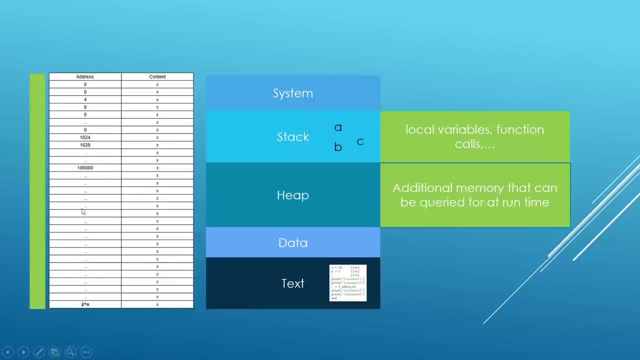 going to load the actual binary of our program so that the CPU can execute it. but we're not going to worry too much about this section in this course because it is out of scope for what we are trying to do here. we are going to focus on stack and hip, because hip is actually going to be. 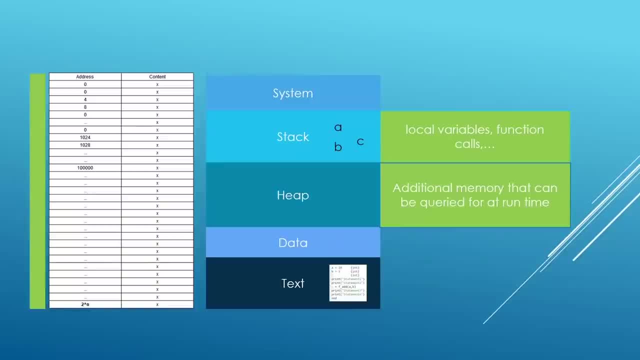 very important from the next lecture when we start talking about dynamic memory, hip is going to be additional memory that you can use in your program if you run out of stack memory, and we're going to see if you are the reasons why you might want to use this as we progress through this course. 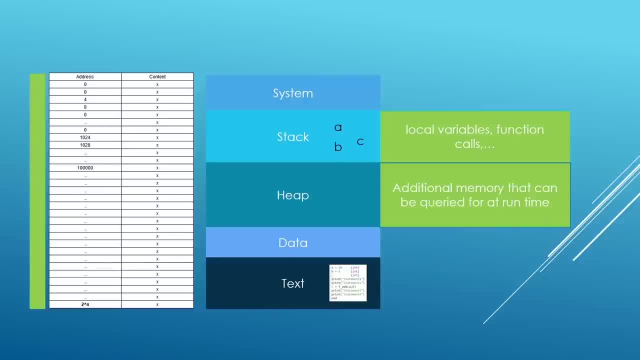 in this chapter. so our memory map is going to have a lot of parts, but the parts that we really care about in this course are a stack and heap. this is really all we set out to do in this lecture. I hope you have a better idea of. 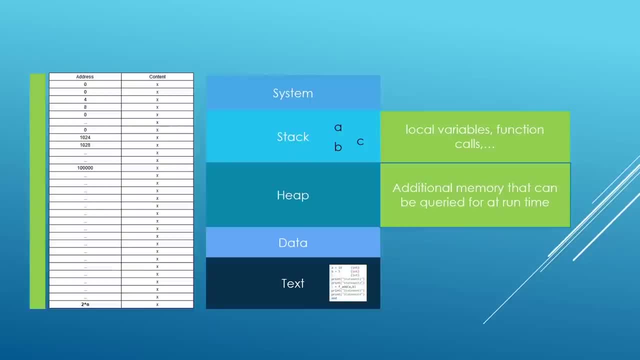 the memory map and how this really works. we introduced another view that you can have on how your C++ program is executed and I hope you have a better idea of the memory system and we are going to start and see how you can work with dynamic memory allocation, which is going to really use the heap, starting in the next. 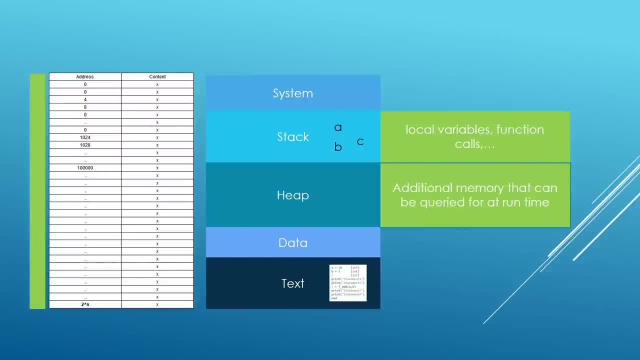 lecture. go ahead and finish up here and meet me there. in this lecture we got to start and learn about dynamic memory allocation and this is a technique we can use to start using hip storage that we have in the memory map of our C++ program. we can use that to get additional memory. we can use and do. 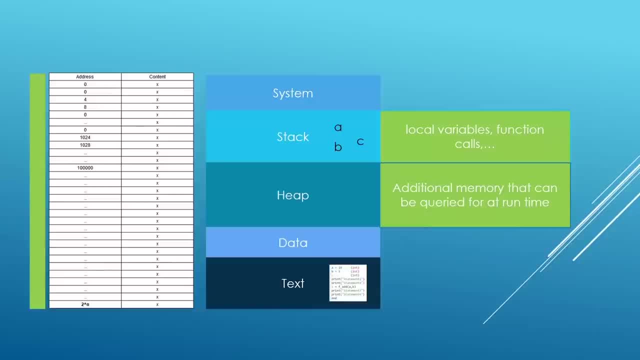 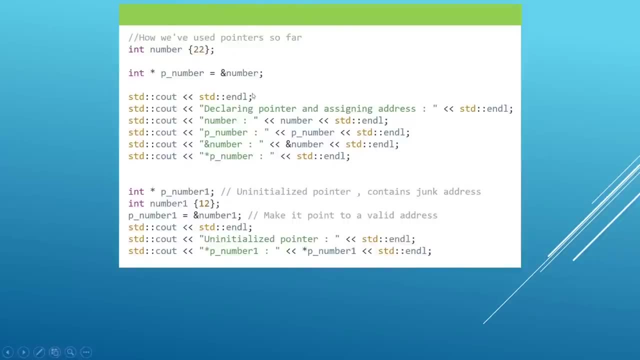 stuff if stack memory is isn't enough for our purposes. this is how we have been using pointers so far. for example, we have a variable, we set up a pointer and we store the address of the variable n, so we can go ahead and use this pointer to manipulate the variable or do all kinds of crazy things if you go down. 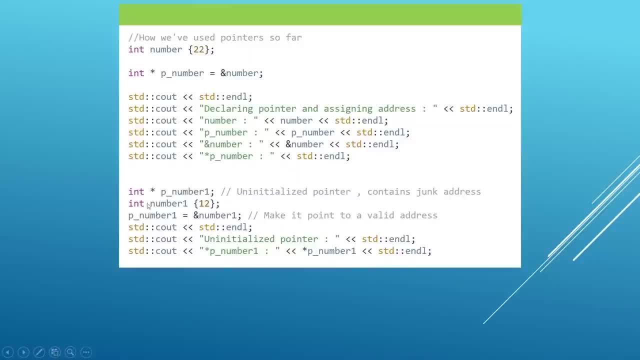 here we have a pointer p, number one, and we have a number one variable and we can store the address of number one into this pointer. it's really the same thing like we have on top here, but the pointer is not initialized at declaration here and you have to make sure you put invalid data and one. 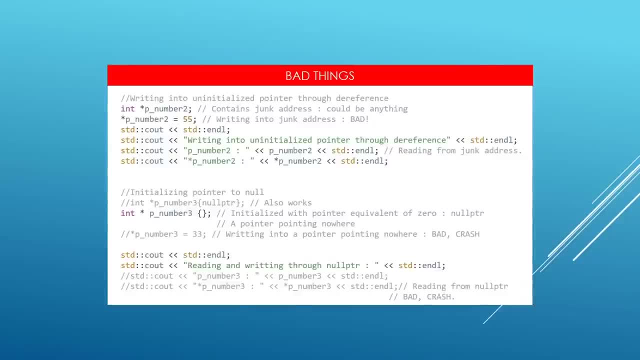 thing i haven't really stressed enough is that it is really bad, really bad, to try and use a pointer that is not initialized. for example, here we have p number two, which is a pointer. it is not initialized, it contains junk, and we try and write into it. 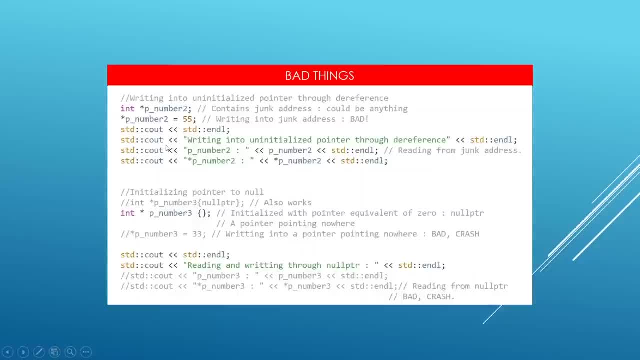 okay, so i'll try to think about what we really are doing here. this is a pointer that we have set up- we haven't really initialized that- so it's going to contain whatever address is possible. it can contain an address that is used by another program. it may contain an address that is being 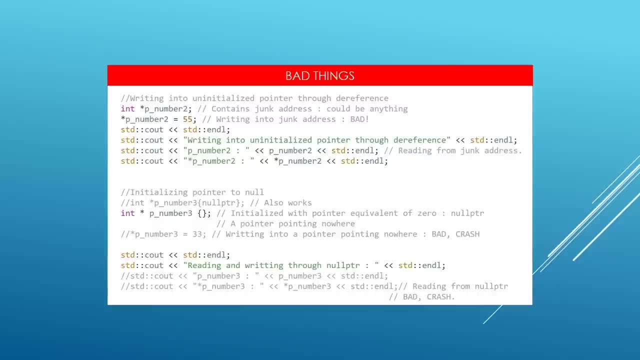 used by the operating system. it's not your address to mess with, and here we are actually trying to mess with that by storing n a 55. so this is going to cause a crash possibly, or even you may have a connection. so we have a point in the box that is going to try to construct a 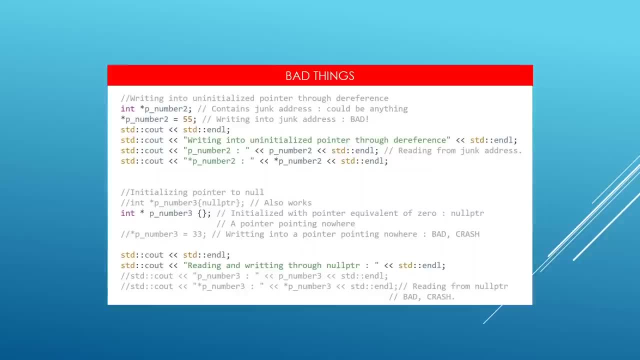 corrupt data that is being used by other people, so don't do this. another thing is to try and use a pointer that is initialized to null. for example, here we have a pointer p, number three, and it is graced initialized. this is going to initialize it to no pointer, but we are trying and storing. 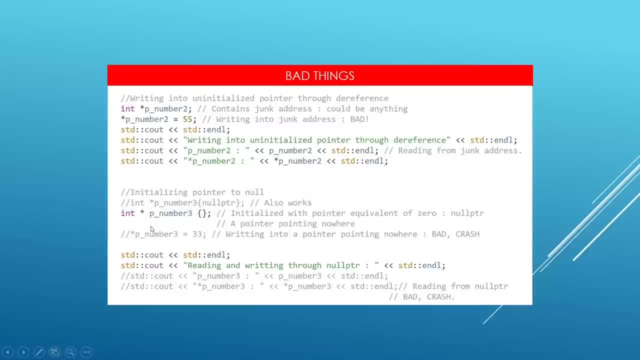 in a value here. so this is also going to be bad. it's not guaranteed what you're going to get. actually, c plus plus doesn't give you any guarantees. this is called undefined behavior. so you're going to get a crash and don't do it as a good practice. the first thing you should do is: 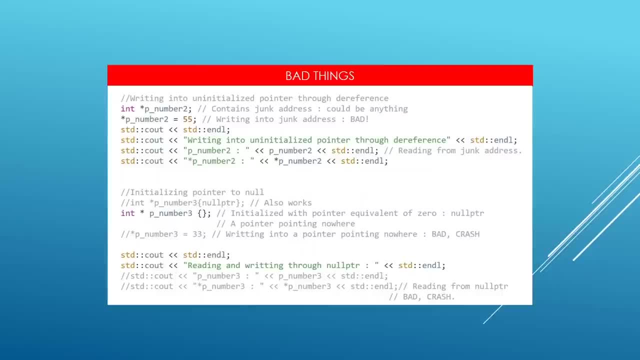 initialize your pointers before you use them. you can initialize them with null pointer and make sure that you are modifying valid addresses into those pointers. if you don't know what is in a pointer, don't use that pointer, because bad things can happen. okay, rule number one: don't try to use. 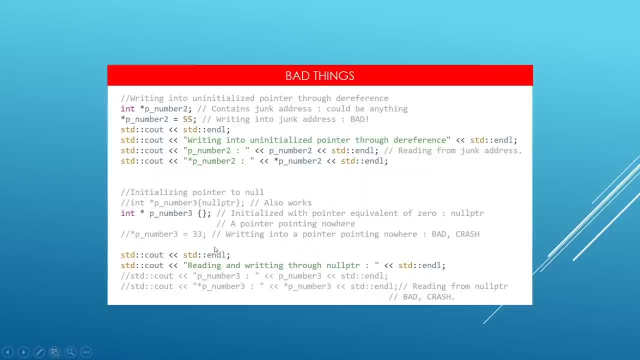 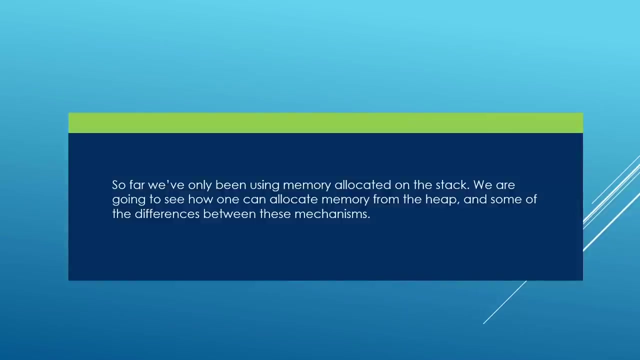 a pointer that you didn't initialize. rule number two: don't try to work with a pointer that is pointing to little ptr. that's going to give you bad things you don't want to really deal with. okay, so far we have been using memory that leaves on the stack section of our memory map. we were 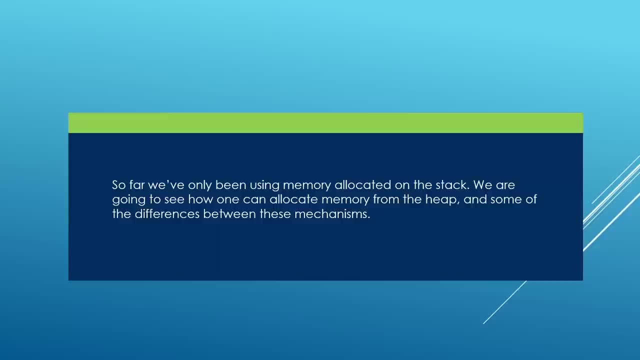 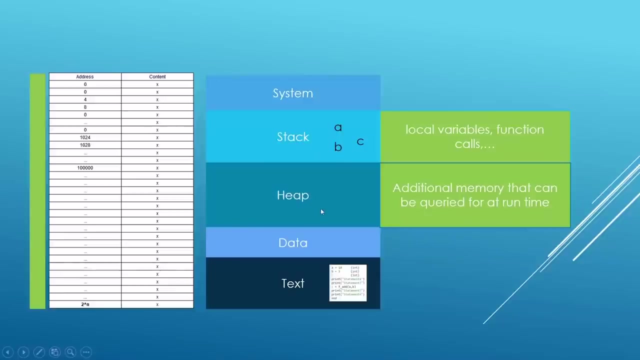 using variables that we have declared in the main function. we were using variables that we have declared inside some functions, and that's all stuff that leave on the stack. now we want to see how we can use the hip. okay, let's take a closer look at our memory map. we have the stack, we have the heap. 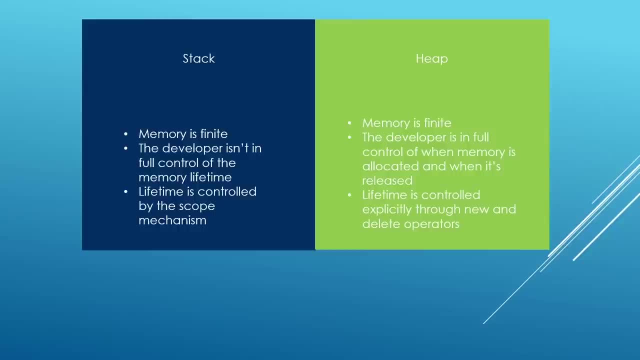 and the differences between these two guys are laid out here. the stack memory is finite, so you don't have infinite memory. but the same is true for the heap. but heap is additional memory that you can use if you don't want to run out of stuck memory. for stack memory, the developer isn't in. 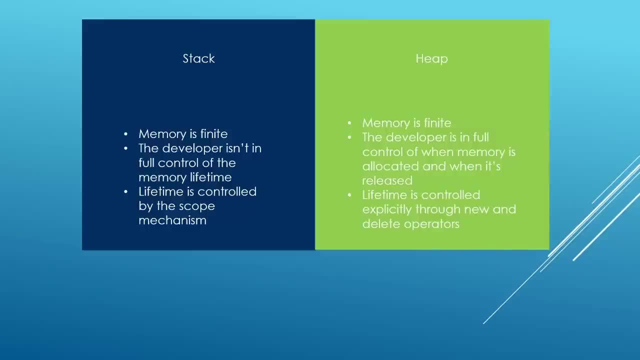 full control of the memory lifetime. so if you declare something on the stack, for example if you say int var1 and you initialize that to 23, you don't control when that variable is wiped out of memory. the variable is going to be killed when the scope in which it was declared is going to. 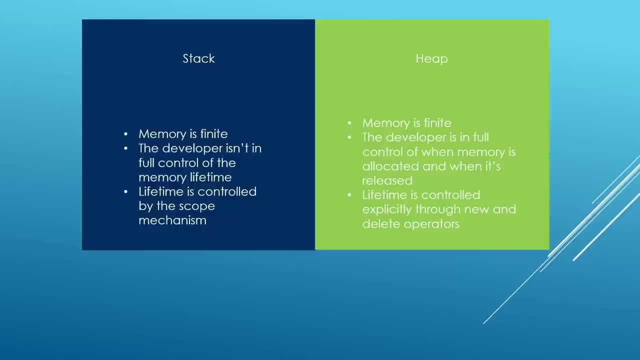 run out and you, the developer, don't really say when the variable dies, and sometimes you really want to control when your variable dies. so this is an example of how you can control the memory. this is a limitation we have with the stack memory. okay, so for stack memory, lifetime is controlled by. 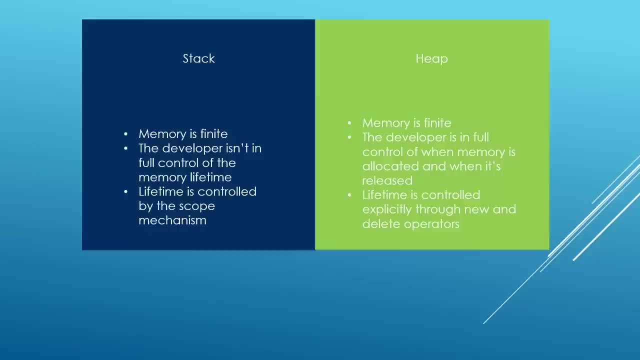 the scope mechanism. we just say that for heap, the developer is in full control of when the variable comes to life and when the variable dies, and this is a benefit you might have with heap storage and you might want to use this, and we're going to see how we can use that in the next few lectures. okay, 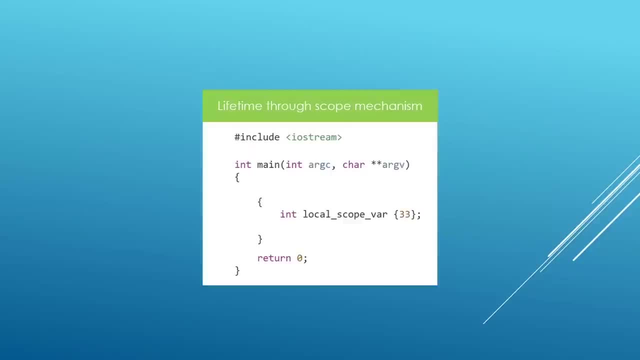 so make sure you understand the difference between stack and heap here. if you look at the example, which is called locus scope var, it is stored within this block delimited by the curly braces, and the variable is going to come to life when this statement is executed, but it is going to die. 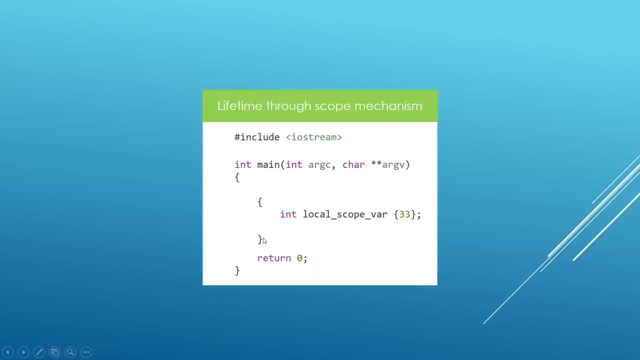 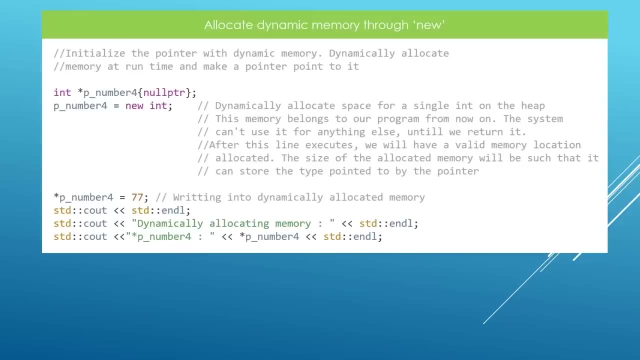 when we hit the closing curly brace here. so the lifetime of this variable is controlled by the scope mechanism, but it is possible to use dynamic memory or use memory on the heap, and we're going to see a syntax you can use to do that. the first thing we want to do. 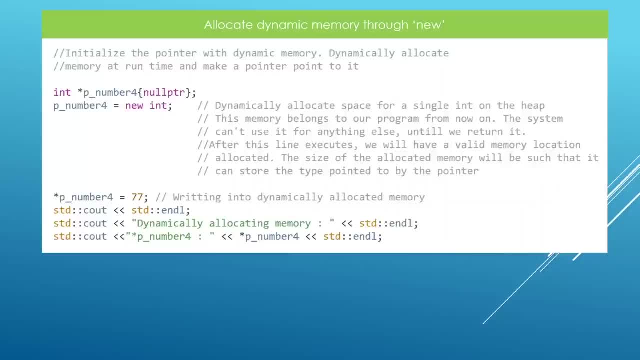 is to set up a pointer that is going to be pointing to that heap allocated memory. the way you do that, you set up a pointer. here we have p number four. we initialize it with null ptr. but what we do to allocate memory is the second statement. here we say p number four and we say 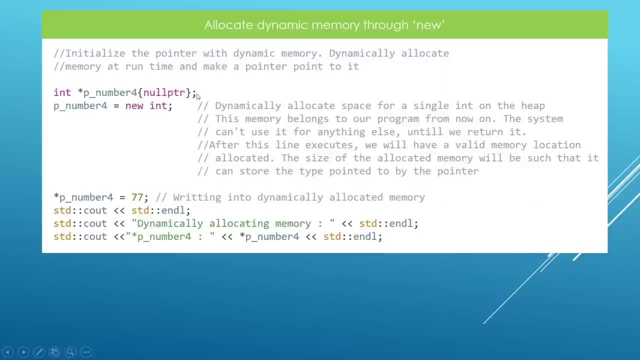 new end. the moment this statement is going to be executed, the operating system is going to allocate a piece of memory on the heap. the memory is going to be large enough to be able to be executed on the heap. the memory is going to be large enough to accommodate for an integer, so it's going to be. 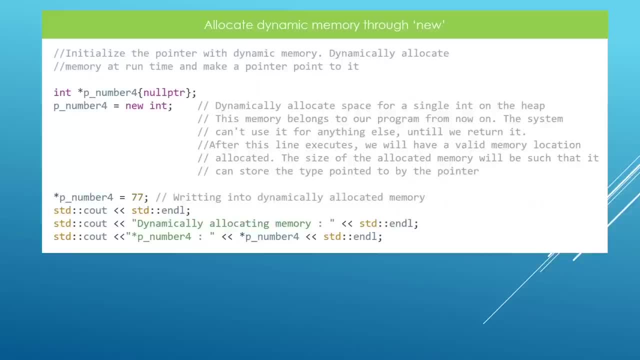 four bytes long and it is your memory. now your program can use it to do whatever it wants and no other program on the system can use this piece of memory. so it is going to be yours until you explicitly return this piece of memory to the system, and we're going to see how you can do that. 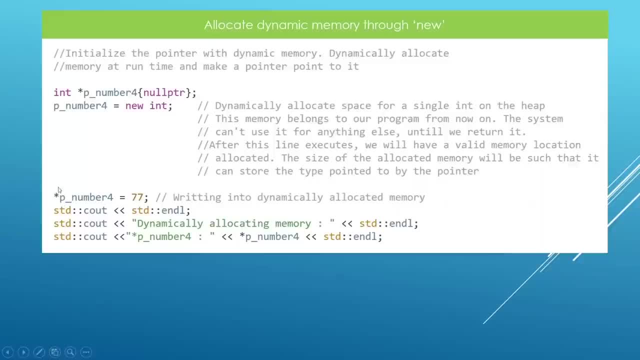 in a minute. once this memory is yours, you can use it. you see, here we are already referencing the memory and the storing gain is 77, and if we're trying to print this out, we're going to have to do the same thing. here we are going to say that the memory is 277. we're going to get it printed. 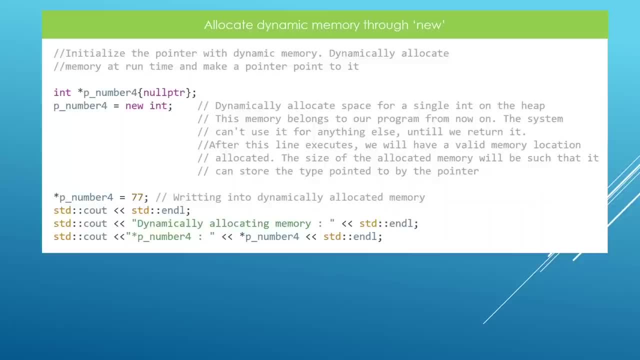 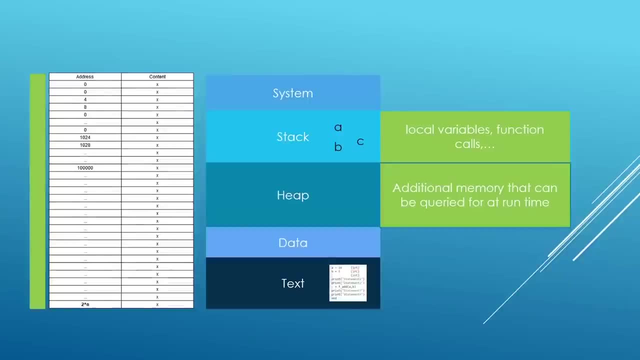 down. okay, this is how you can use dynamic memory, and when you do this, things are not being stored on the stack, things are being stored on the heap. i really hope you understand this, because it is very important. okay, so here is our view of stack and heap. so if you use new to allocate for memory, 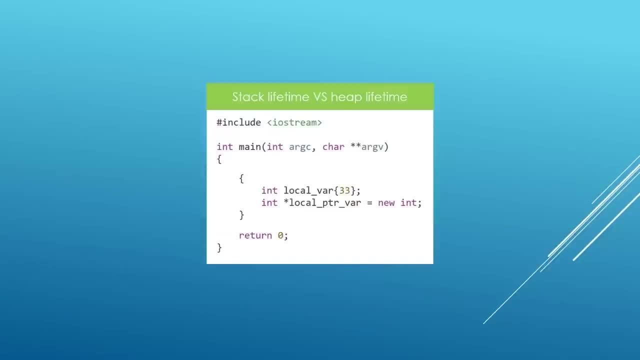 stuff are going to be stored in this heap, section here of your memory map. here is another example to do um. so what we're going to do here is we're going to say: state: this is a variable which is going to be stored in this heap and it's going to come into life when the statement here is executed. 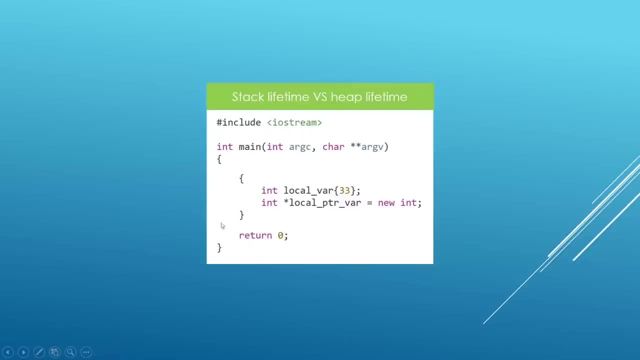 and the lifetime of our variables. docovar, again, is limited to this scope. it is going to come into life when this statement here is executed and it is going to die when we run out of this scope here. so if you try executing code out of this scope, local var is no longer going to be available. you. 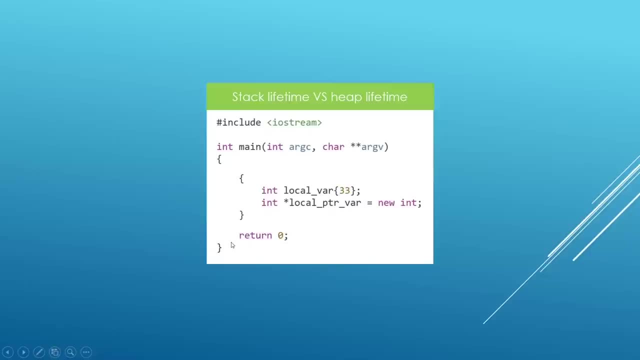 can't use it, but that's not the case for local ptr var, because this is a pointer- it lives on the heap scope. the memory is still going to be yours if you have a way you can access it and use it. you're going to be able to use it and it is going to be yours until. 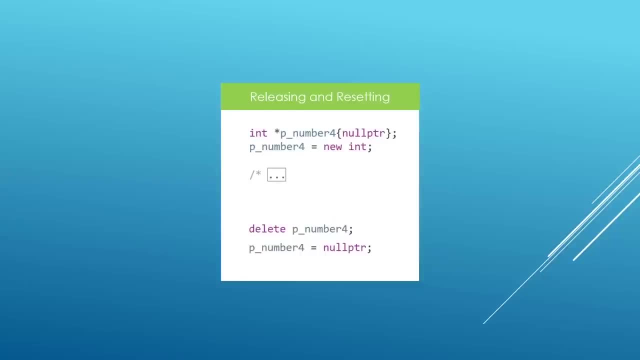 you decide to return it to the operating system. so we have been talking about returning the memory to the system. how do we do it? well, you use the delete keyword in C++. here we have our memory, which is allocated using new, and so the operating system is going to give us a new piece of memory. it is going to be: 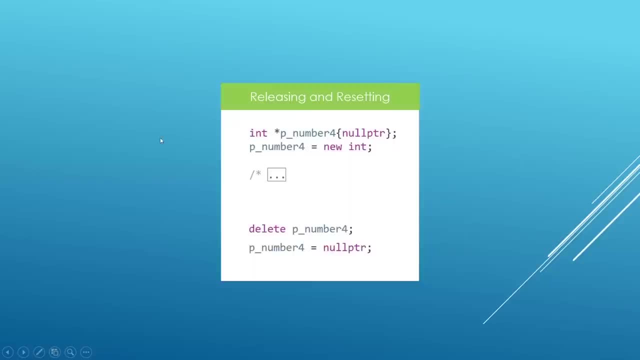 4 bytes, because we're going to store in an integer and we are going to be pointing to that memory through P number 4. here we can use this memory however we want to, through the referencing, and do all kinds of crazy things, and when we are done with this memory, we are going to say: delete P number 4 and this: 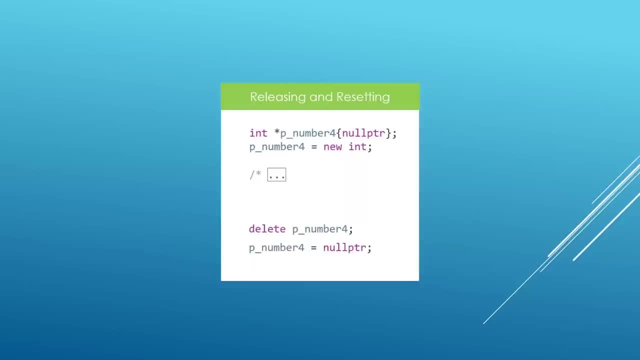 statement is going to return the memory to the operating system. the memory is no longer going to be ours after this statement, and a good thing to do after that is to return the memory to the operating system. so we are going to you release your memory is to reset it to no ptr so that other people know that you don't really. 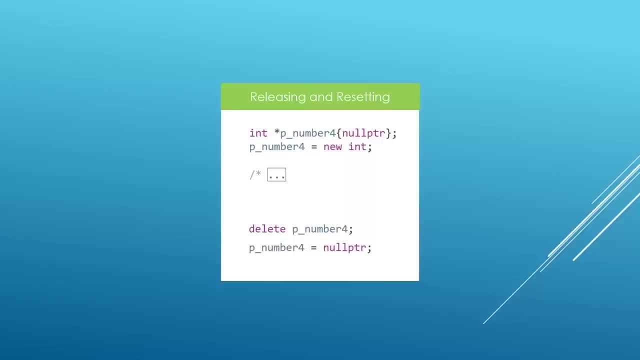 have any valid data in that memory, because if you try to use a deleted memory section, bad things are going to happen. that's not going to be your memory. we're going to fall into the same problem of trying to use an uninitialized piece of memory. don't do that. so whenever you release memory, also reset it. 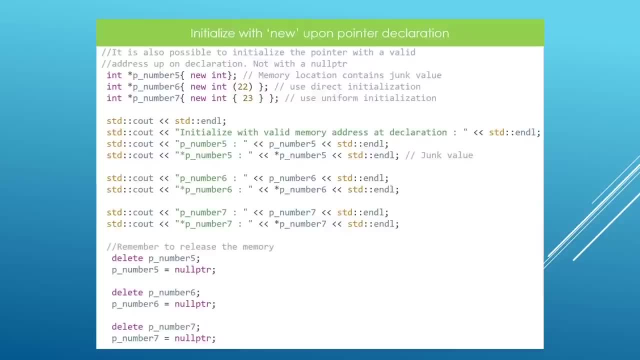 to no ptr. to play it safe, we can also initialize our pointers with dynamic memory when we declare them, and this is how you can do it: we say p number five and we initialize it with new, and this is going to give us a new piece of memory on the heap and it is going to be pointed to by p number five. 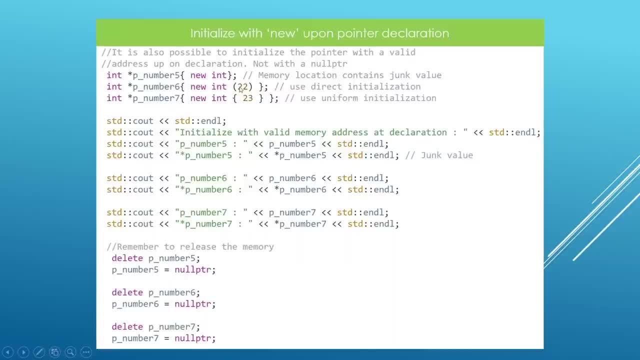 we get the same thing here, but here we are just putting in new values in p number six and p number seven. the memory locations on the heap are going to be containing twenty two and twenty three for p number six and p number seven, and here we have a few examples. 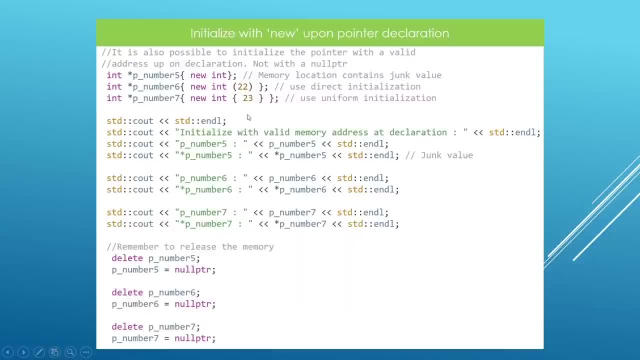 of how we can print the contents of these memory locations on sddc out and after you are done using your heap memory, you're going to release it using the delete keyword and you are going to reset that to no ptr to really play it safe. this is how you should use dynamic memory. 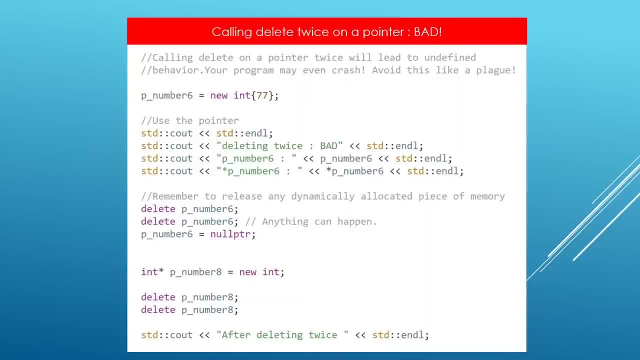 allocated on the heap. another thing you should know is that it is really bad to call delete twice on a pointer. so here we have a memory location that we allocate on the heap, we store this in a pointer and, uh, we are trying to use it here in sddc out reading: 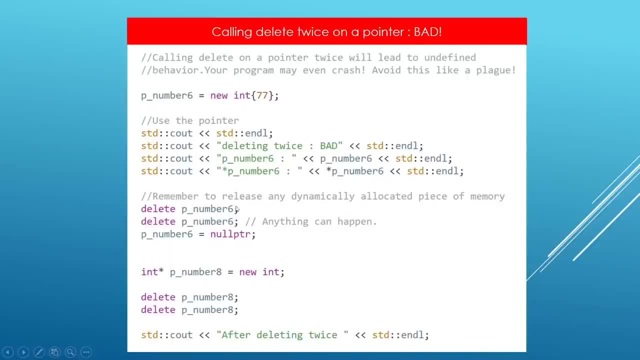 whatever is inside. and if we delete it for the first time, that's going to be cool. it is going to be returned to the system, but if you try to delete it for the second time, you're going to get a crash. don't do this. this is really bad. okay, now that we have a slightly better memory location. 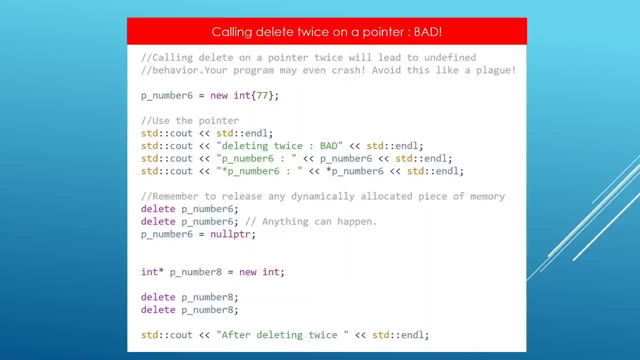 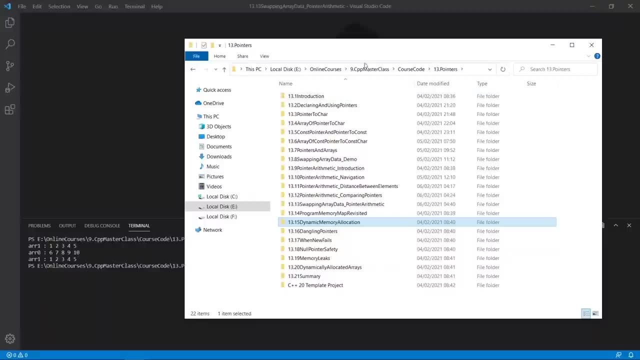 our ptr has gone especially well thanks to gri. Often, a lot of people prefer to have extremely clear idea about pointers and dynamic memory allocation. I think it is time we went to vision studio code and actually played with a few of these concepts. here we are in our 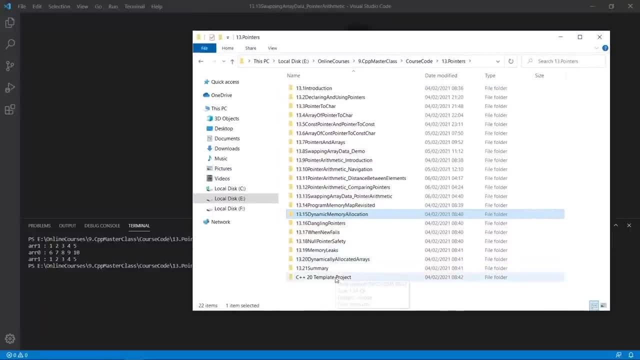 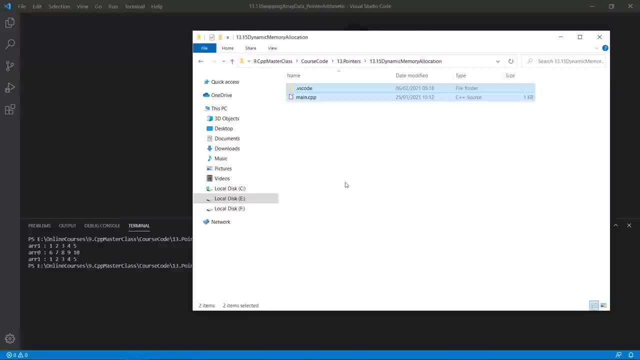 working directory. the current project is dynamic memory allocation. we're going to grab our template files and we're going to put them in place. dynamic memory allocation: let's do that and we're going to open this in vision studio code, the first thing we're going to. 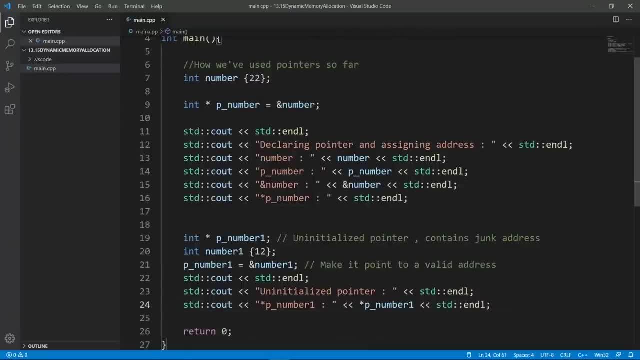 do is review how we have been using pointers so far. we have got the build and understands it very clearly. visual studio code is one step ahead of sleep Hardware Menu, which has been. we have been using them like this: we had a variable stored somewhere on the stack again. 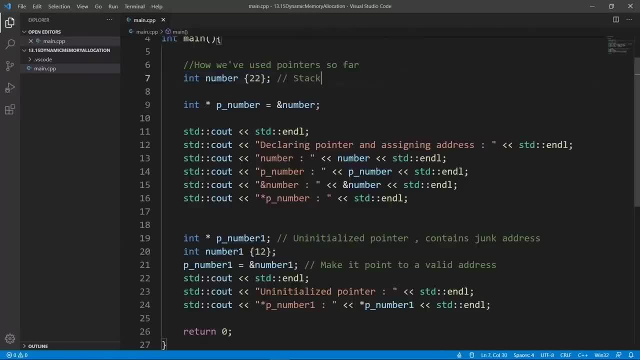 this is a stack memory that we are using here and we stored addresses of some variables in our pointer or something like this, and we could go through the pointer to manipulate that memory location, for example. we can print the address of that memory. we can even do reference and print. 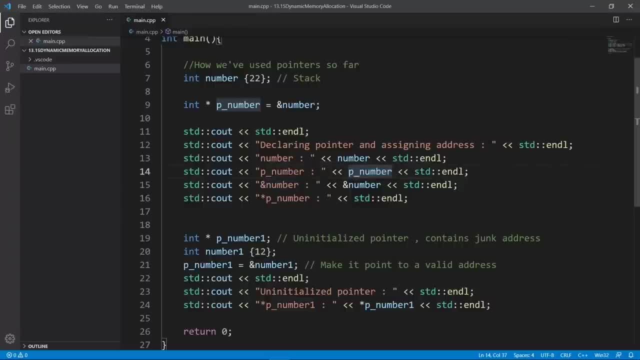 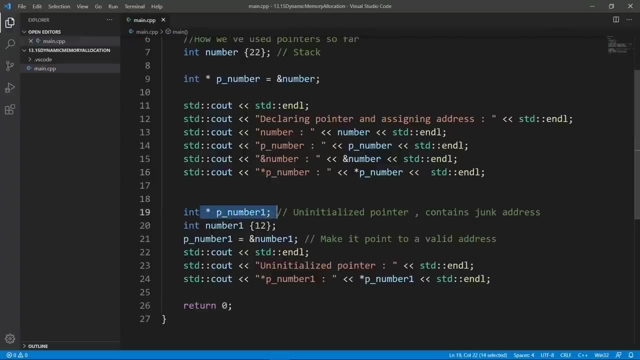 the value in here by doing something like we do here and we are not printing here, so let's say that and say p number. we can do something like this and we have been doing this quite a lot so far. we can also have a piece of memory that is uninitialized and we store the address of some. 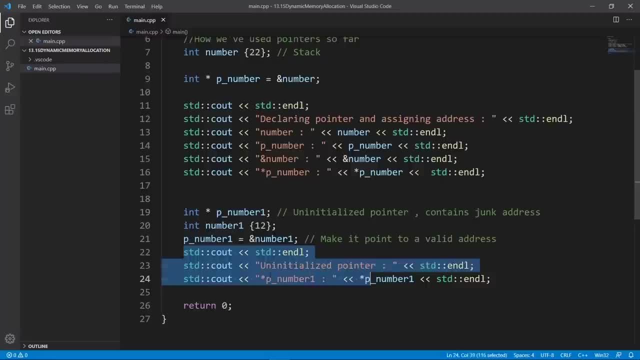 variable in that piece of memory and we can do the same thing. for example, if we print p number one, we're going to get the value 12 printed out here and we could run this. so let's try and do that. we're going to bring up a terminal first and close this pane so that we have some breathing. 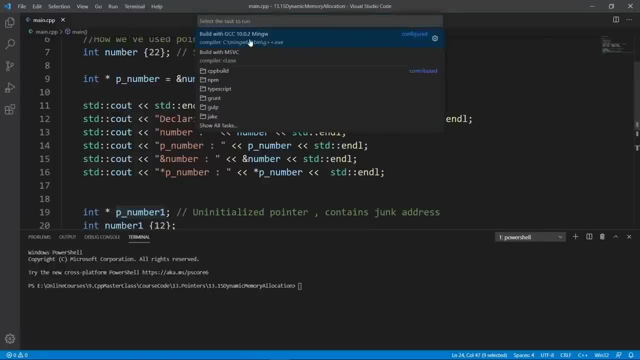 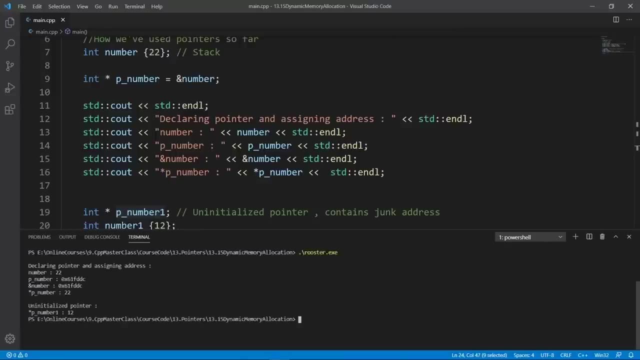 room and we are going to build with gcc like we always do. we're going to build successfully. i'm going to clear and run rooster and we're going to see that we have these things printed out here. the variable we have in here is 22, so we're going to get that if we print the variable directly. 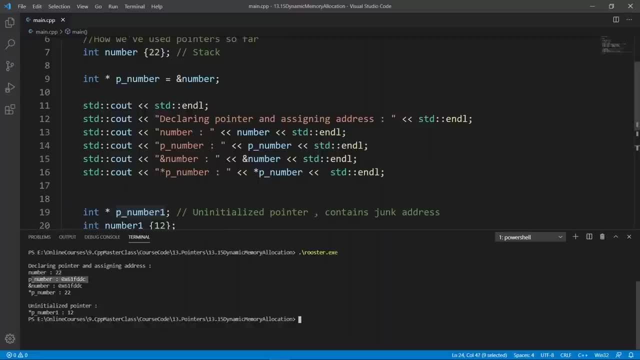 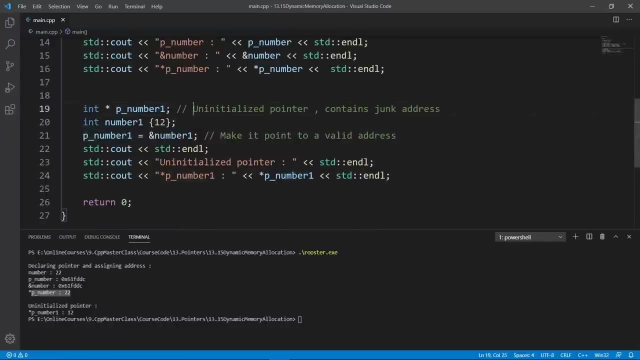 if we print pointer, we're going to get the address printed out. we can also go through the address of operator to print the address of this variable here. but we can also print our value through dereferencing our pointer and we can get access to it here. down here we have a pointer that is not initialized, so it will. 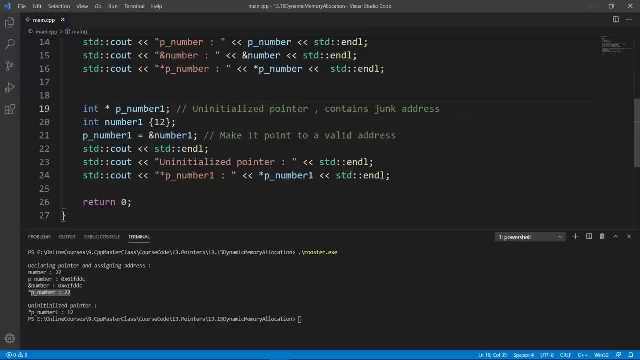 contain a junk address that you shouldn't really use. but we're not going to do that because we're going to store in the address of number one here and we can manipulate the value here through the pointer using the reference operator here, and if we print this p number one, we're going to get 12. 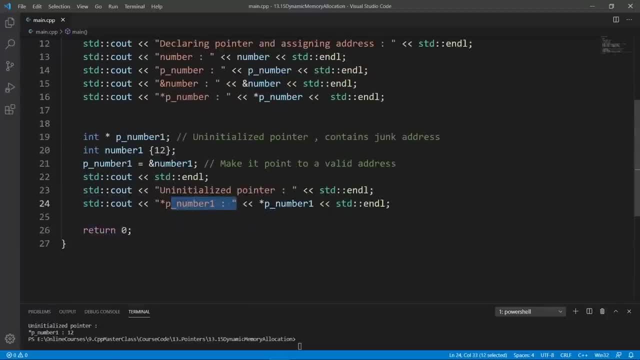 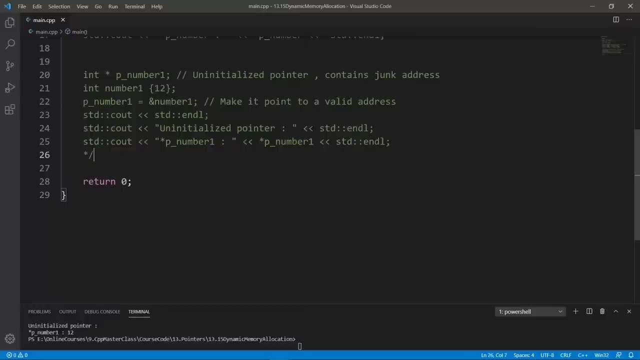 pointed out. this is pretty cool, okay, so this is how we have been using pointers so far. let's comment this out, because we're going to see some other things. okay, before we really look at how dynamic memory works, we are going to show you a few bad things you need to be aware of, so 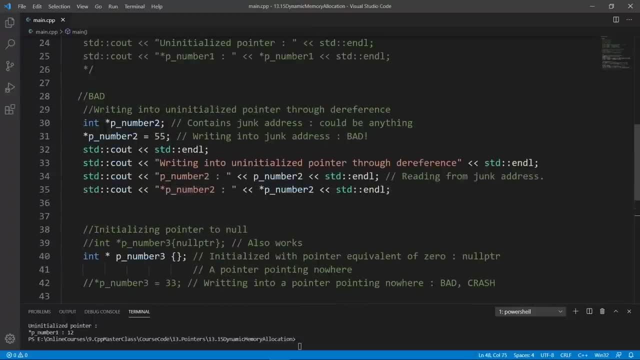 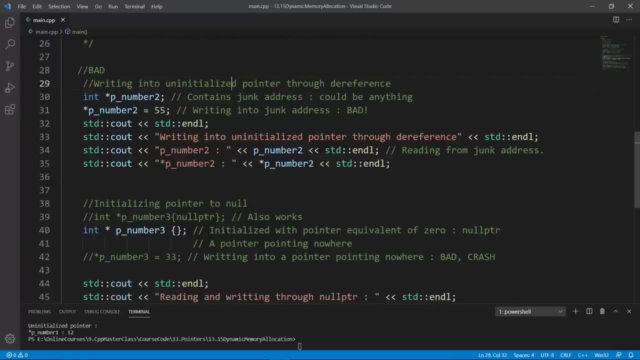 let's put in a piece of code for us to play with, and here we are saying that writing into uninitialized memory is really bad. so here we have a pointer. it is uninitialized and we are trying and directly writing to it through the referencing and this is going to 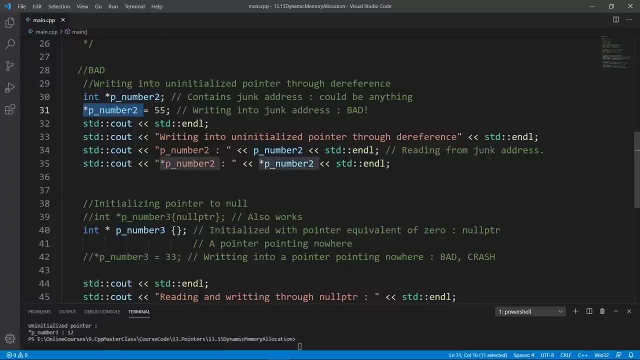 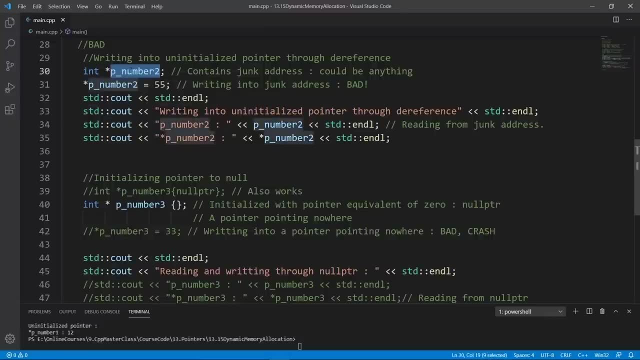 be bad. you see that visual studio code is not complaining. it thinks that we know what we are doing here and it's not going to warn us. but this pointer could really be pointing anywhere, including operating system specific memory, and here you may be trying to modify things that your operating system is going to need. so clearly the operating system is not. 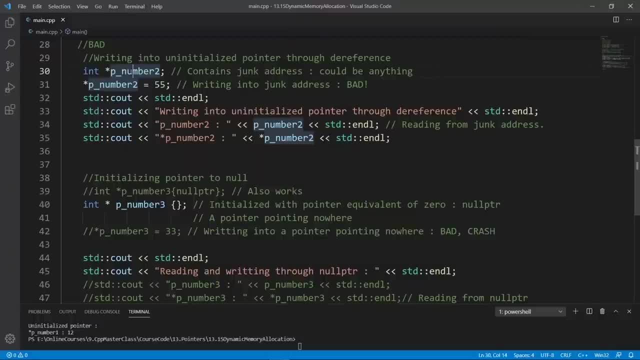 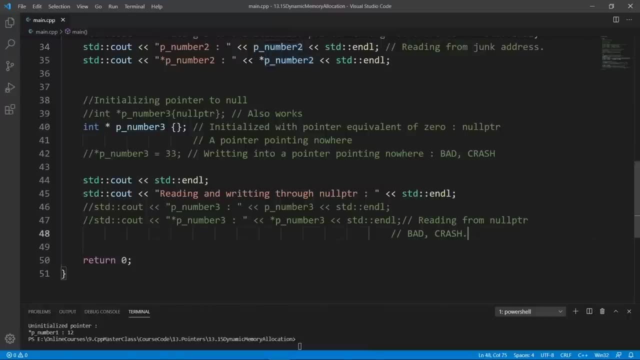 going to be happy about this and bad things can happen to this program. so now we have this memory location, we're going to try and write into it and we're going to see what happens if we run this program. for now, let's try and take this little section here and comment it out, and we 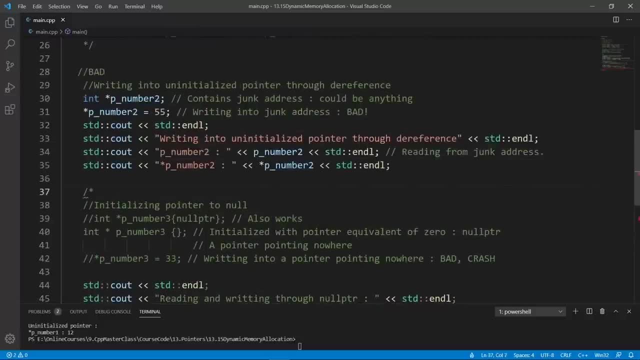 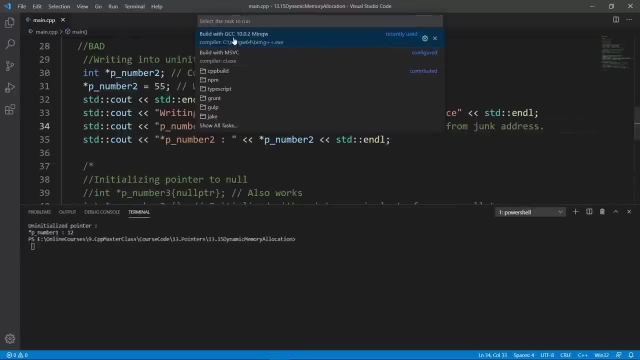 want to see what happens on the program here, the code here that we might want to run. let's try and build that with gcc. we're going to run the task. to do that, the world is going to be good. you see that we don't even get a compiler error. and if we're trying to run rooster, you see that the 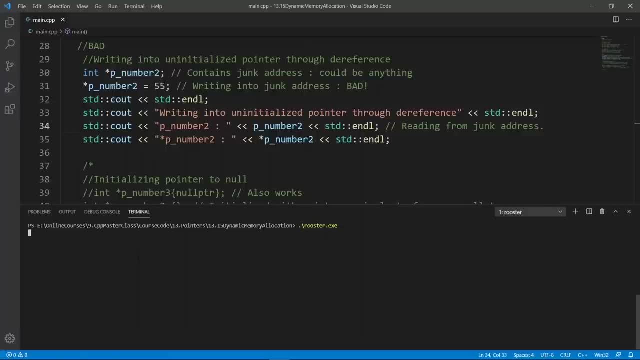 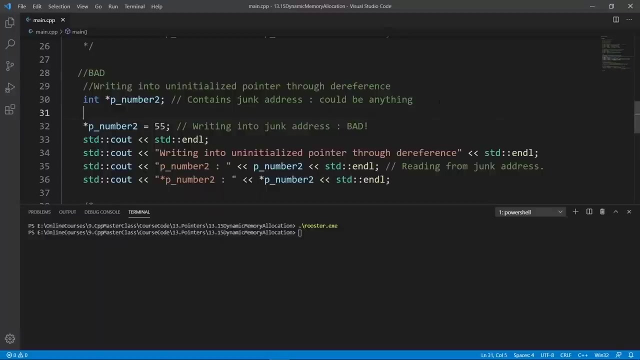 program is going to try and run. you know the operating system is going to say: this guy doesn't know what they are doing and i am going to close them. you see that it's not even running this statement here. let's go on top here and put in an stdc out statement so that we can really see. 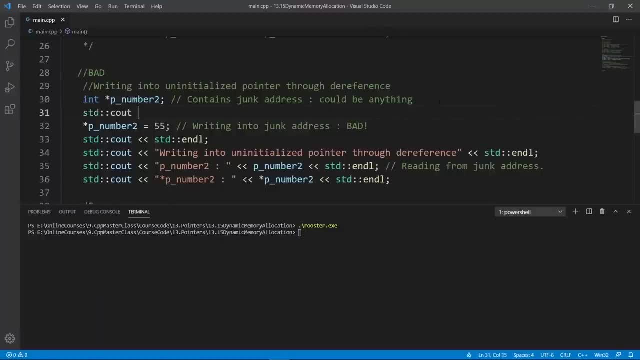 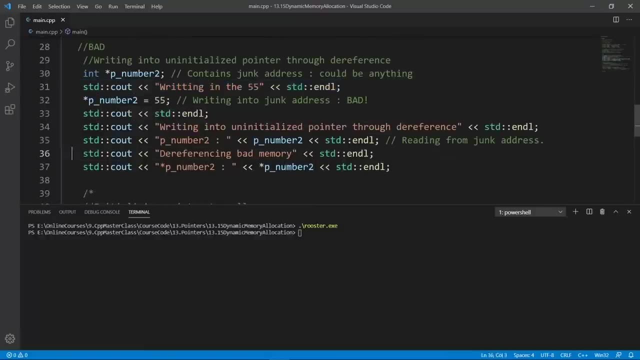 where this program is failing. let's say that stdc out writing in the 55. okay, so this is what we have. we have a few statements added in and we want to see if we actually get to run these two things to see where the program is actually failing. we are going to build it again with gcc and we are going to 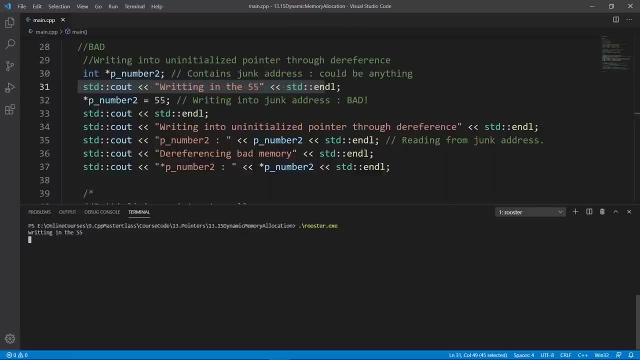 clear and run rooster. you see that it's going to say writing in a 55. but this statement here is going to fail because we are trying to write into memory that is not ours and the operating system is going to stop us. so our program is crashing and it is terminating before it even runs the things that 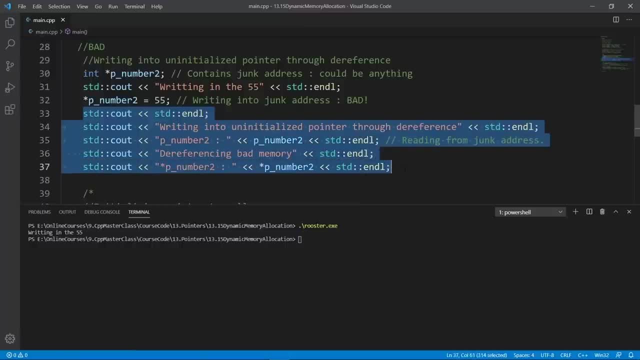 are down here. hopefully you can see how bad this is. you have designed your program to do things, but it is going to stop without having done any of the other things that you have designed below. so this is really bad. and another bad thing is that you might have 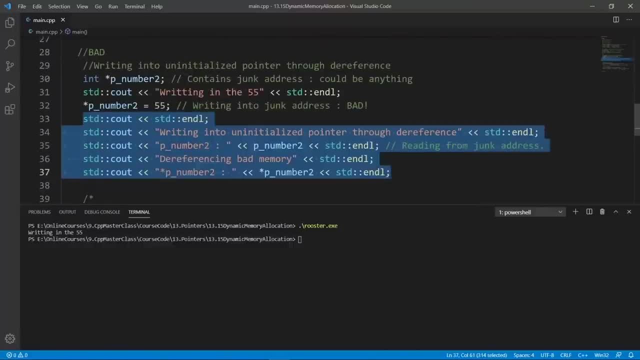 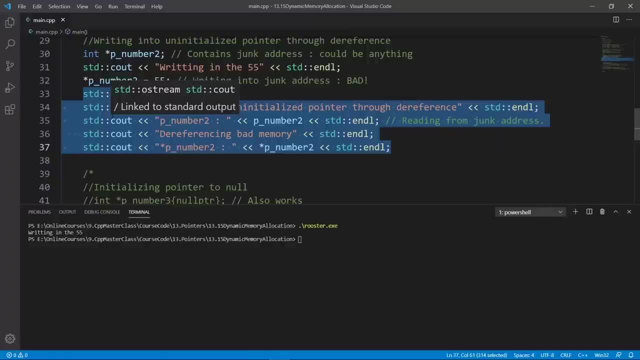 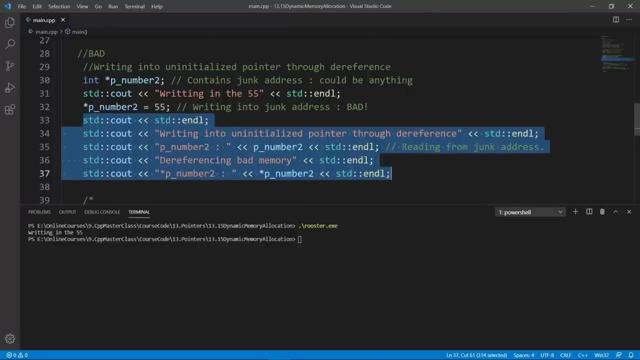 allocated some dynamic memory beforehand and your program is going to end before it even releases that memory properly and returns that to the operating system. so this is bad. you don't want crashes in your programs and don't ever try and use and reference memory that you haven't. 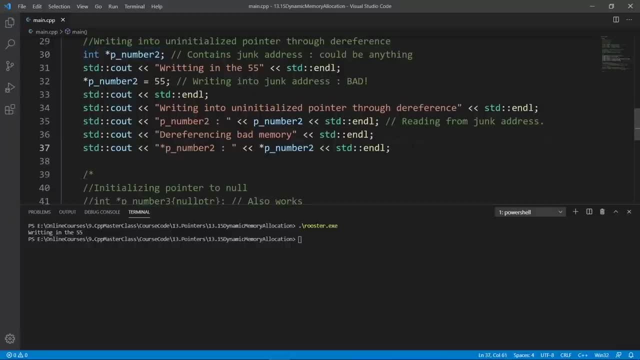 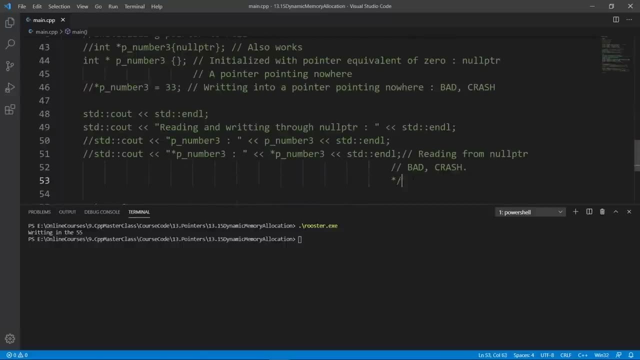 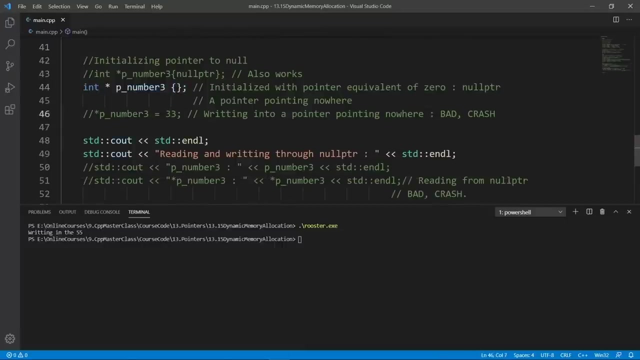 initialized. this is one bad thing. we're going to comment this out. i hope you really know how bad this is and we're going to go down again and and comment what we had done here. and uh, it's going to be another bad thing because we are trying to write into memory. 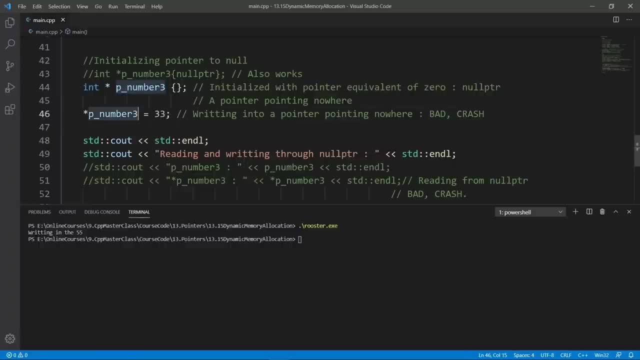 initialized to null ptr. okay, here we have a pointer. it is called p, number three, and it is initialized with no ptr. you can think of ptr as an address that says: i don't have any valid thing in me, don't use me. that's what no ptr is saying. so we have the pointer initialized to ptr. 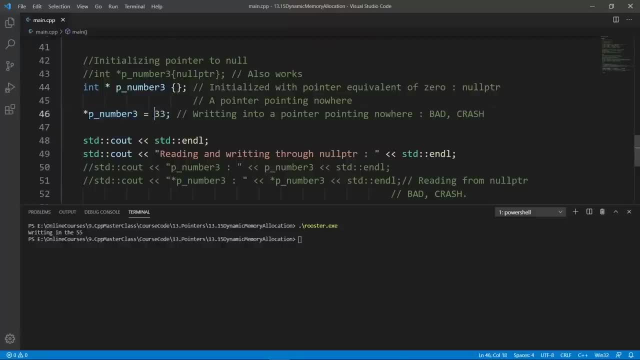 but we are trying to store something in here and you can imagine how bad this is. this is memory that isn't really valid. the memory itself is saying: i don't contain anything valid, don't try to use me. and if you try to use it, bad things are going to happen. so if we try and compile this, 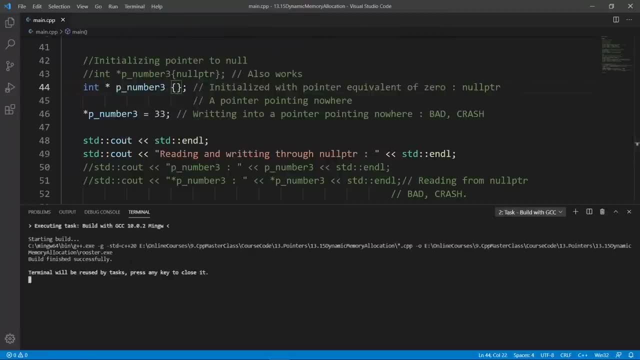 program it is going to compile. the compiler is not going to stop us to do something like this, and these are some things you need to be aware of in c++. but if we try to run it, you're going to see that we are also going to get a crash again. let's try and put a statement in front of. 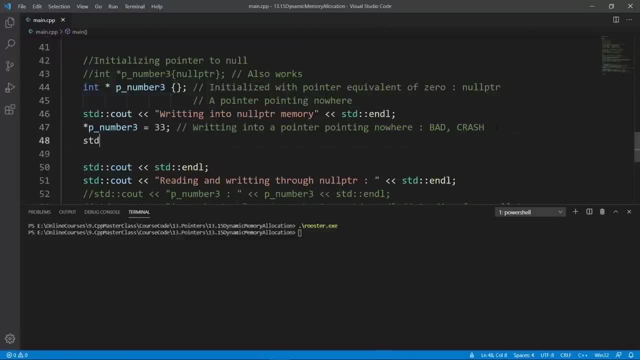 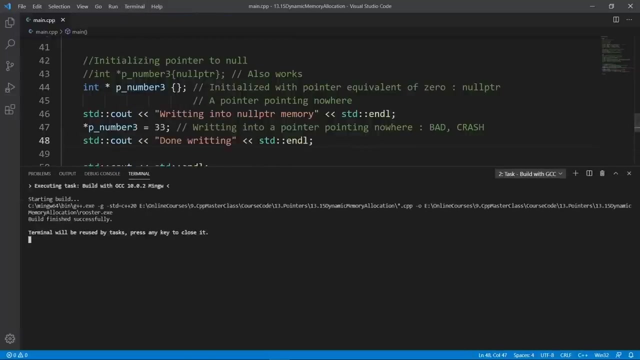 this failing line and below this line i can say: done writing and i can do std endl here and weld the program so that we can see which std statements run and which not, after our program crashes. so we're going to clear the weld is good and run rooster, you're going to see it's going to. 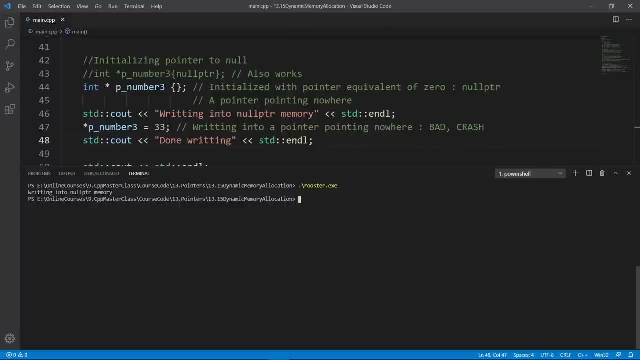 say what it's doing. it's going to try and fail. you're going to see. it's going to say what it's doing. it's going to try and fail and the operating system is going to kill this program because it is crazy. it is doing what it. 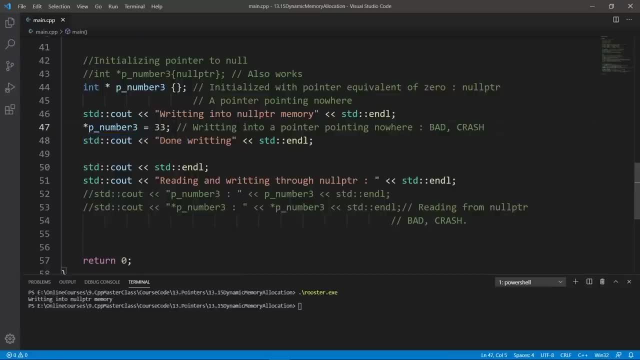 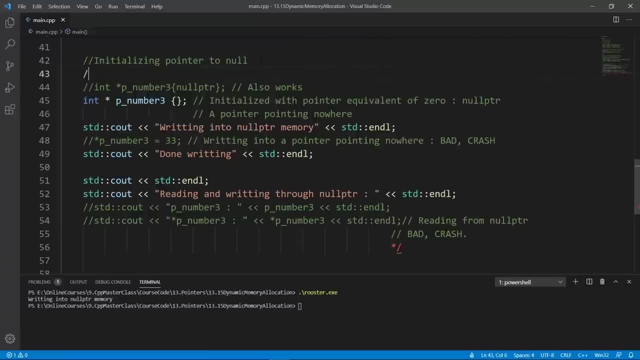 shouldn't really be doing so. this is something bad. don't do it be aware of this thing? okay, we're going to comment this out and actually look at how we can dynamically allocate memory from the heap, and we're going to put in a piece of code to play with that. it's not really complicated. we have a. 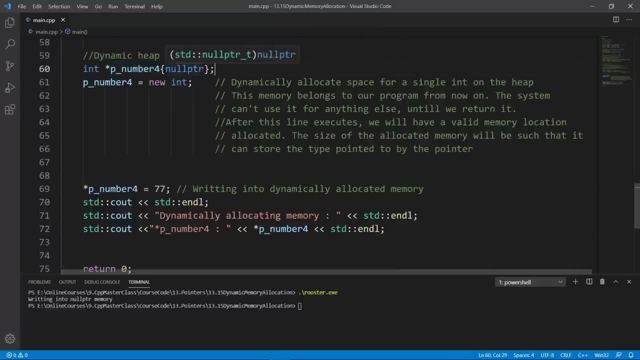 pointer. we initialize it with no pointer to say that this pointer doesn't point to anywhere valid, don't use it. and we are calling new. and when we do this, the operating system is going to give us a new piece of memory on the heap. this piece of memory is going to have the size enough to contain an end, so it's going to 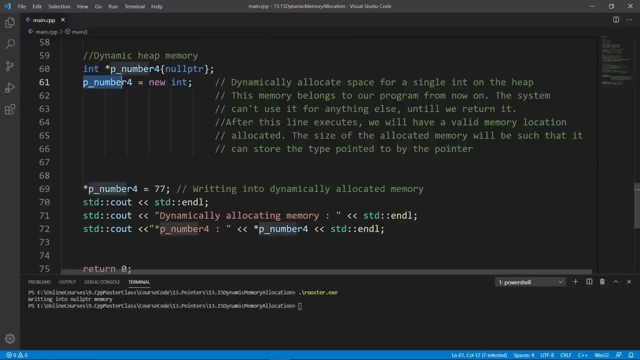 be four bytes in memory, and we are going to be pointing to that piece of memory using the p number four here. this is what we are trying to say here. the moment we do this, we own this piece of memory and nobody else on the operating system can use it, so that's something you should know. 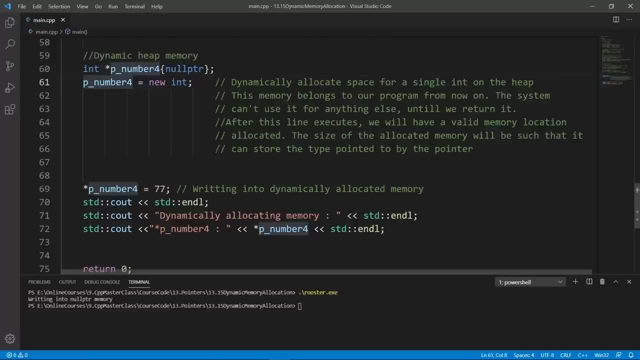 once you have it, you can manipulate the memory and you can use it to do whatever you want to do, and we are going to print it through the pointer here. so here we can go through the, the reference operator, and store in the 77, and if we print it out, we're going to get that printed out here. 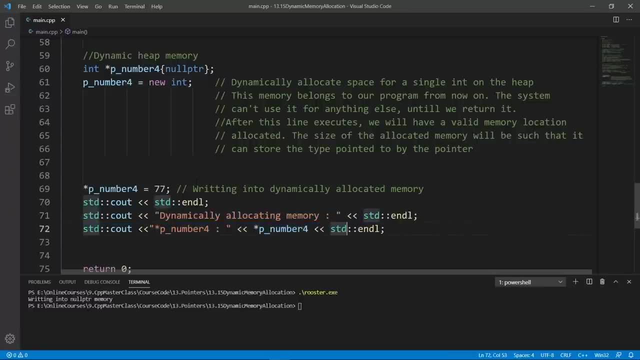 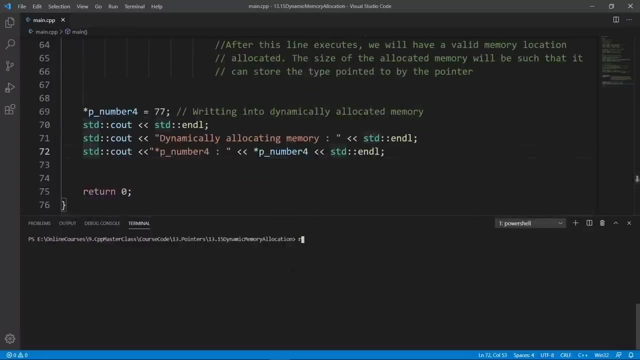 okay, this is really cool. this is the first time we use heap memory and i am excited about showing you these things. we're going to try and build this program and the build is going to be good and we are going to clear this and if we run rooster, we should see a 77 printed out. let's do. 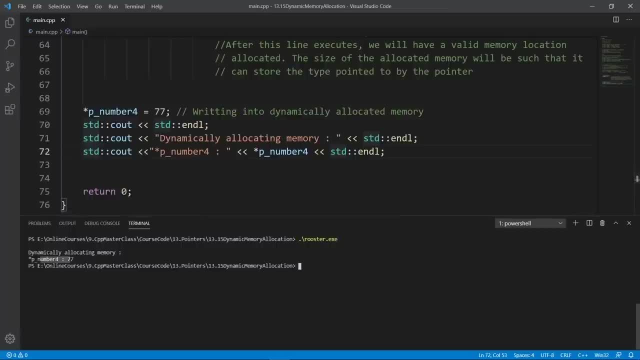 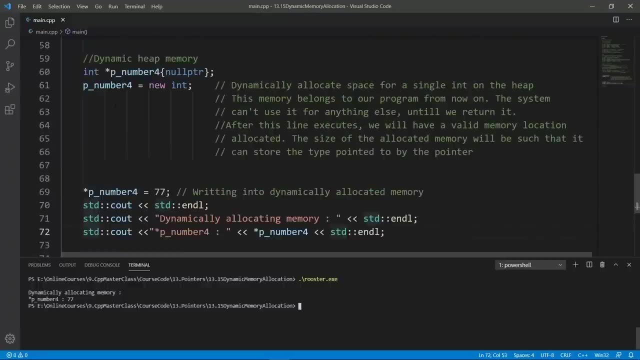 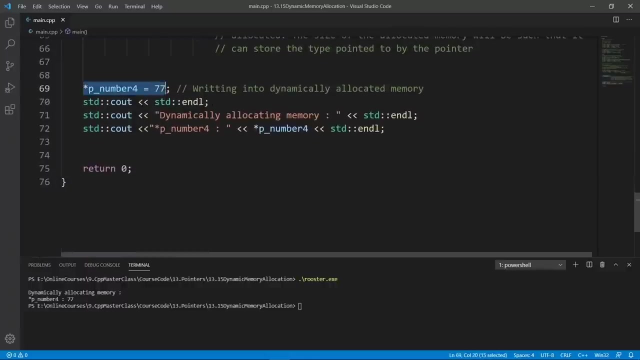 that we're going to get our 77, but this 77 is stored on the heap now. it is not stored on the stack, and this is really, really cool. we can control when this variable comes alive by allocating memory on the heap, and we exactly control when this variable dies, if we want, and we're going to see how we can. 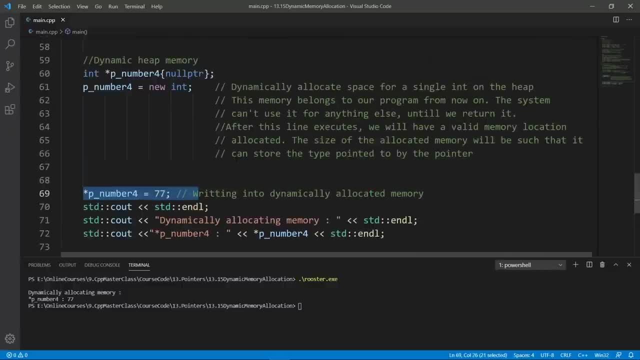 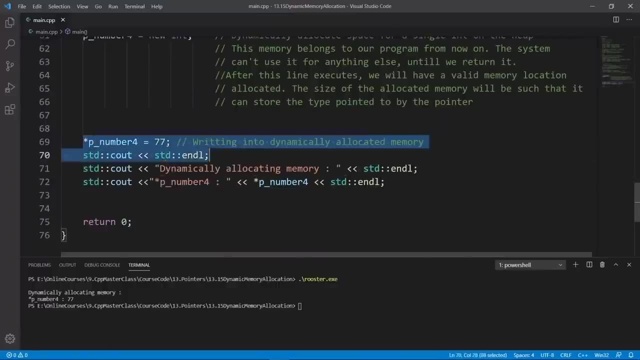 kill this variable from memory. but for now, just take a moment and appreciate how cool it is to be able to allocate stuff on the heap. it is really cool. now that you have used the memory, it is really time to return it to the system because we have no more use for it the way you. 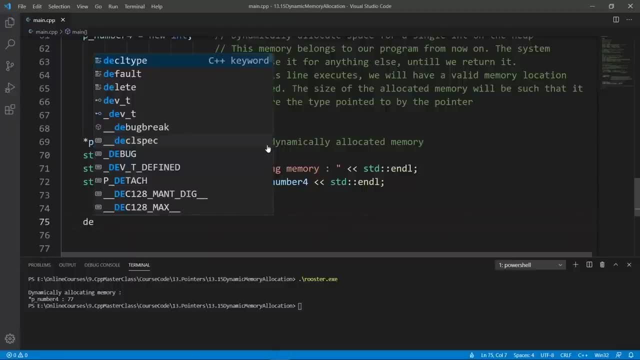 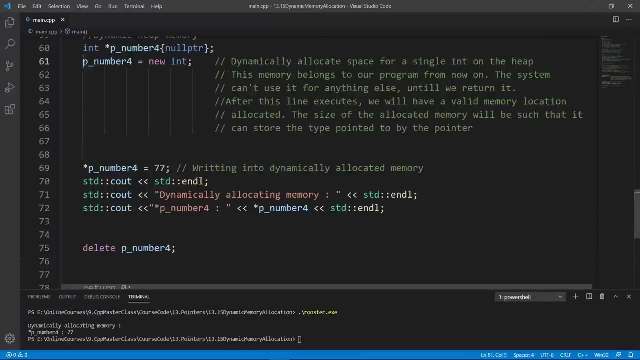 release memory to the system is to call the delete keyword and say the pointer pointing to the memory that you are trying to release to the system. so we're going to say p number four here. let's bring this down a little bit so that you can see the entire story. so we have a pointer here and it 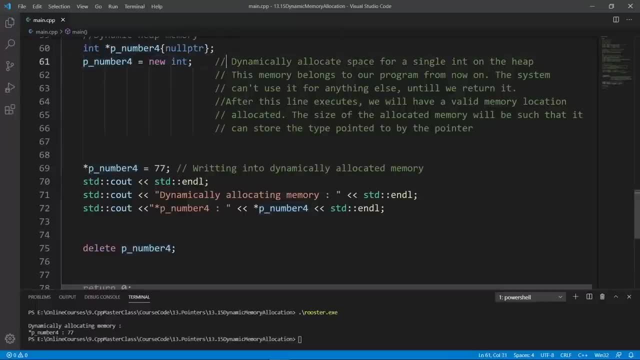 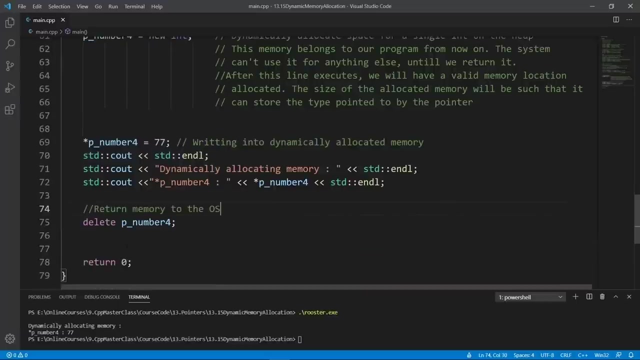 is pointing to dynamically allocated memory from the heap. this memory is four bytes large because it stores an integer. we have it dynamically allocated, we use it here and it is time to return it to the operating system. okay, i hope this is clear the moment you call the delete. 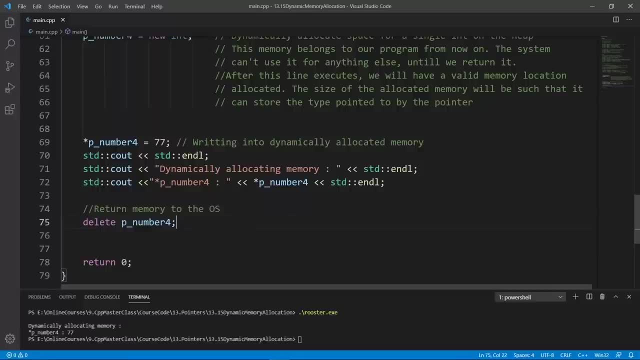 keyword. now the memory is going to be containing some junk and you don't want to really use that anymore. if you try to use it, it's not your memory, you're going to run into trouble. so, for example, after we delete this memory, if you're trying to use it, i'm going to show you here. i think i can. 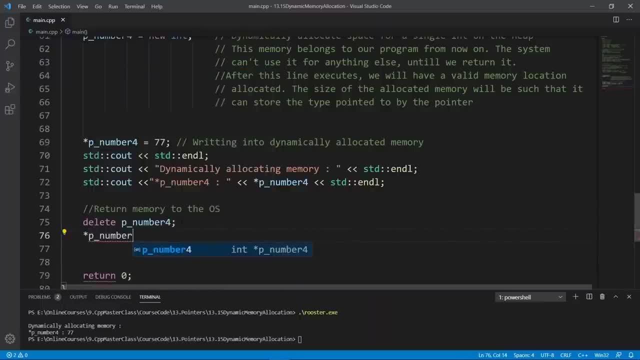 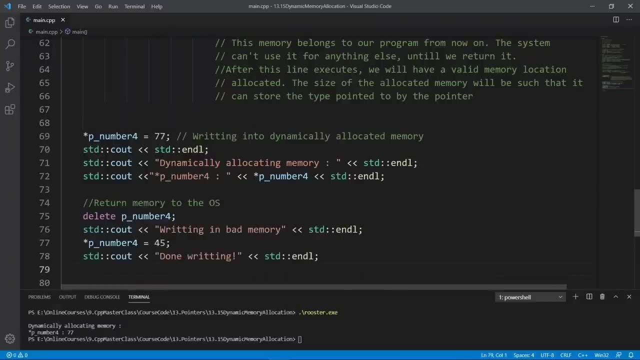 let's see if i can do that. so i'm going to show you here. i'm going to show you here. i'm going to say p, number four and um, storing something. notice that we are using the reference operator and let's try and put in a 45, why not? so let's build this with gcc, as we always do. it is going to world. 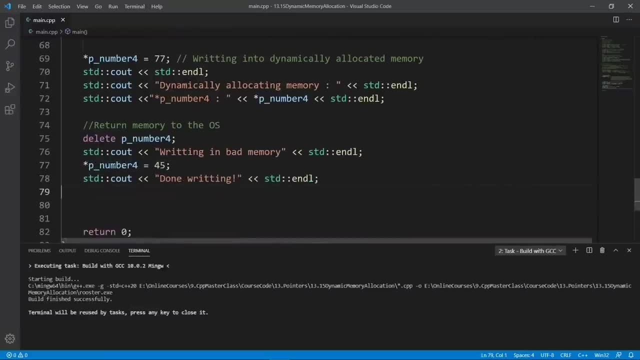 compiler is not going to stop you from doing something like this: writing into memory that you have already released to the system, but we're going to see what happens. so run rooster and it is going to say done writing. but you see that the program has really crashed because here we are trying to write into memory that we don't really own and 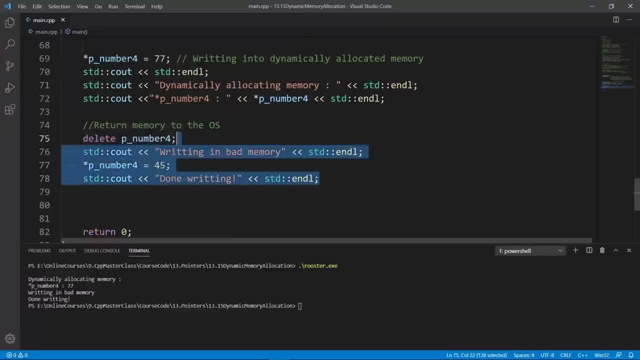 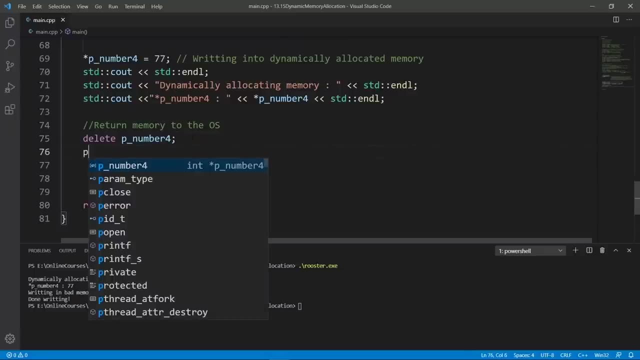 this is bad. don't do this. so the moment you delete the memory or the moment you return the memory to the operand system, it is good practice to reset that memory to no ptr. so we're going to say p number four and make sure it contains no ptr. at least when we do this, other people have a chance. 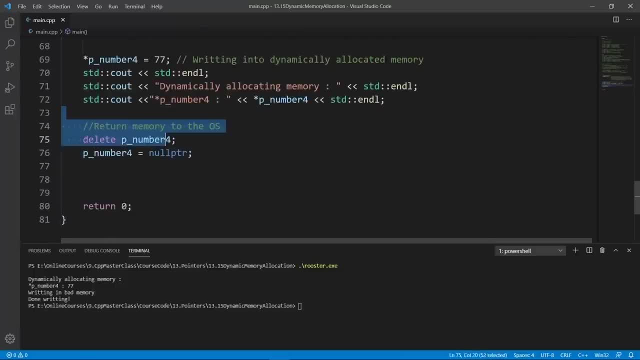 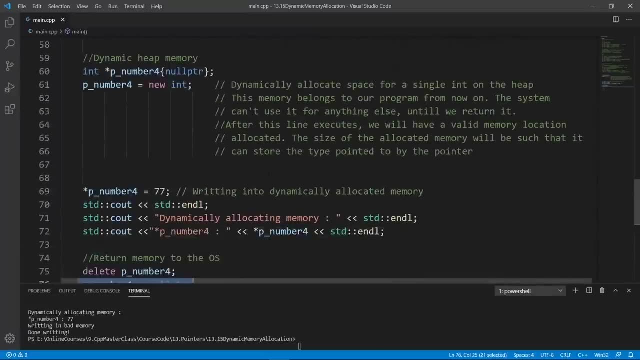 to check and see that that's the way it's going to work. of course, this is going to work for the valid memory before they use it, that's the use of resetting your memory here. so this is something you should do again. the flow to use dynamic memory is really simple. you set up a pointer. 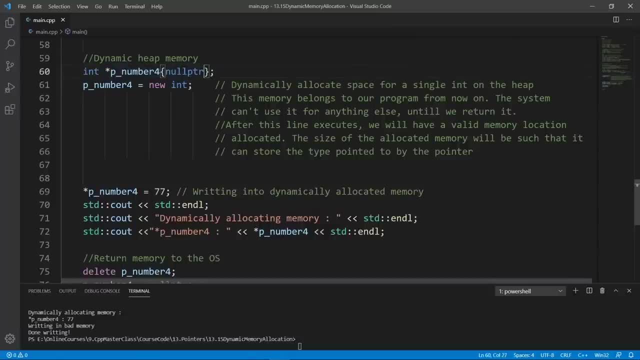 that is going to point to your memory. you're going to allocate the memory from the heap using the new operator. you're going to specify the type you want to allocate memory, for the operating system is going to give you that memory and you're going to be pointing to that memory with your pointer. 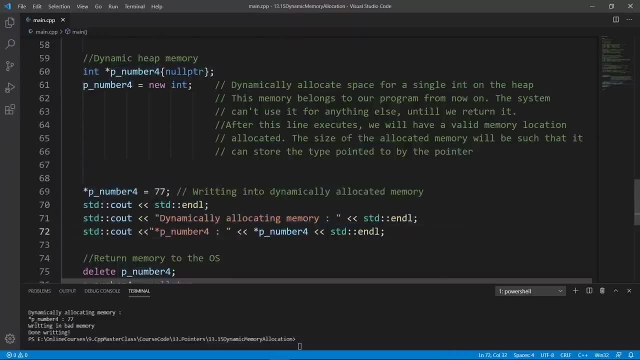 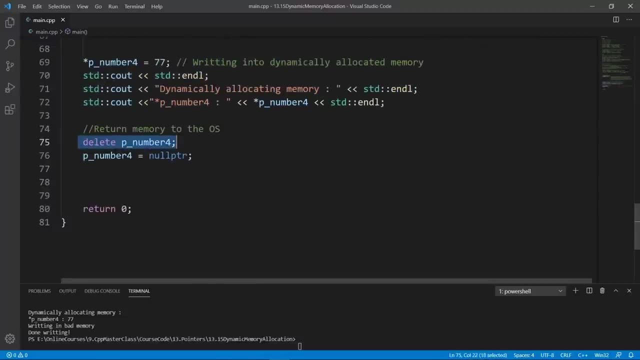 you are going to manipulate that memory using your pointer and doing all kinds of crazy things and after you are done with that memory, you're going to release it to the operating system and please, please, remember to reset your pointers after you have deleted them, like this that's going. 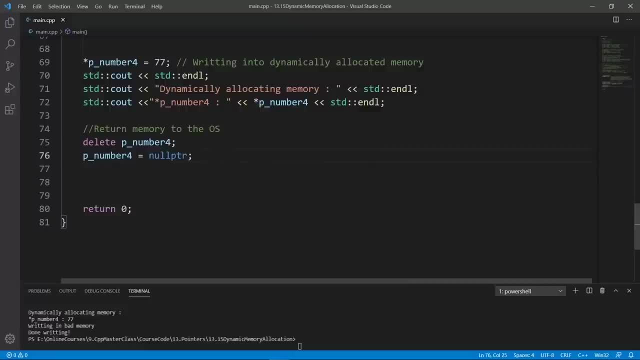 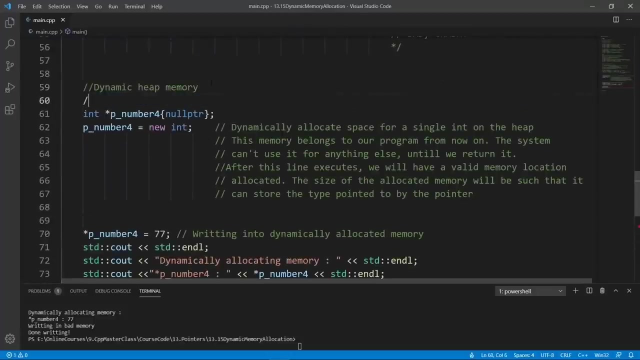 to make your life a whole lot easier, and other developers are going to thank you for doing this when they get to use your code, because your code is going to be much safer to work with. okay, let's call it a day this out and show you another example of what cool things you can do with dynamic heap memory. 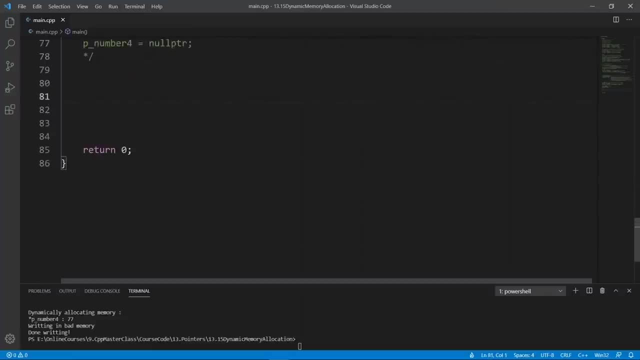 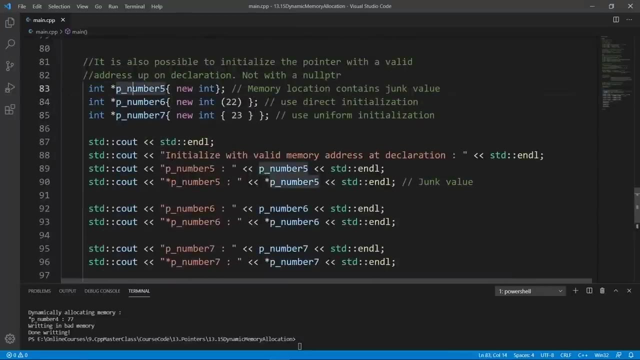 we're going to go down and put in a piece of code and show you that you can actually dynamically initialize your pointers at declaration. this is something you can do. the first one is not initialized, so it's going to contain junk value p number five if we try to. 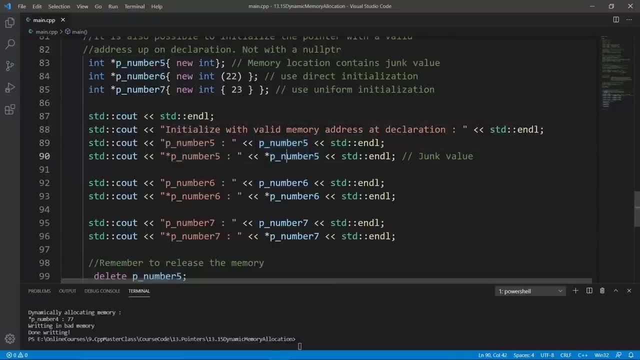 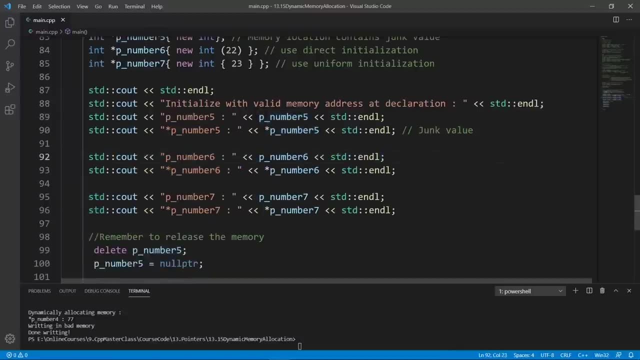 print it. we're going to get some junk address printed out- p number six- we're going to reference it and print the value inside. so we're going to see that and we can do the same thing for p number six and p number seven after we are done using the pointers we are going to release. 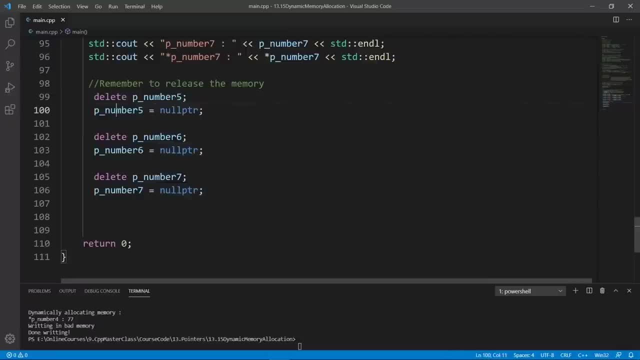 the memory here and notice that we are resetting the pointers to no pointer, to say that they don't really contain anything useful. don't use them. make sure you have something valid in before you use them. this is the meaning here. if you're trying to run the program, you can guess what we're going to. 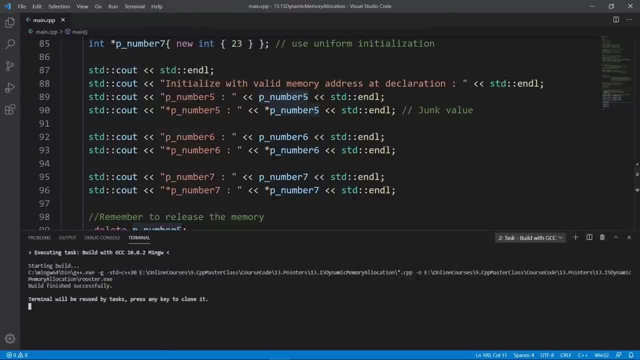 see. so try and guess. and uh, we're going to build, we're going to build successfully, we're going to clear, clear, not clear, and we're going to run this program. we're going to run this program. we're going to run this program and we're going to see that p number five contains some junk address. okay, and. 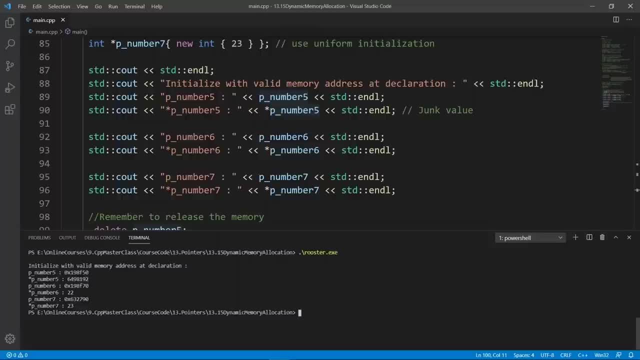 if we try to dereference it, we're going to get a junk value. this is really not useful. don't use this value because you didn't put this value in in the first place. you're going to see that p number six is going to point to some other address, but we're going to have a valid value inside because 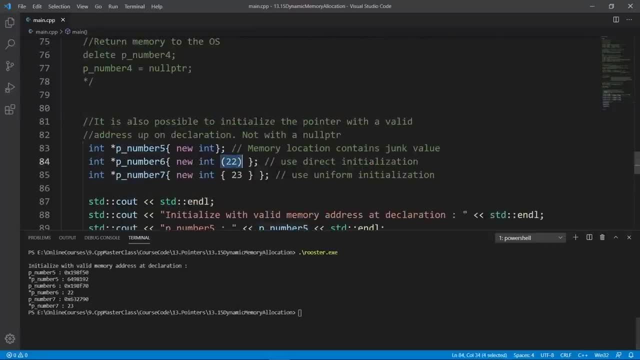 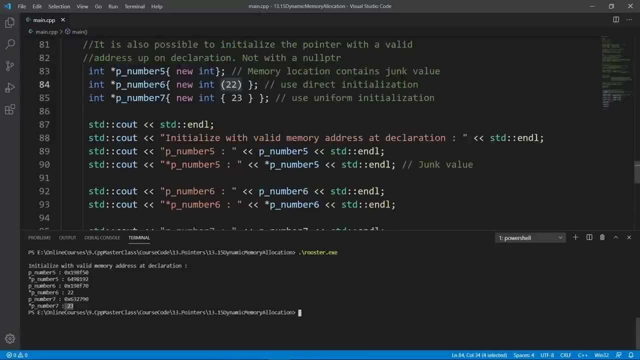 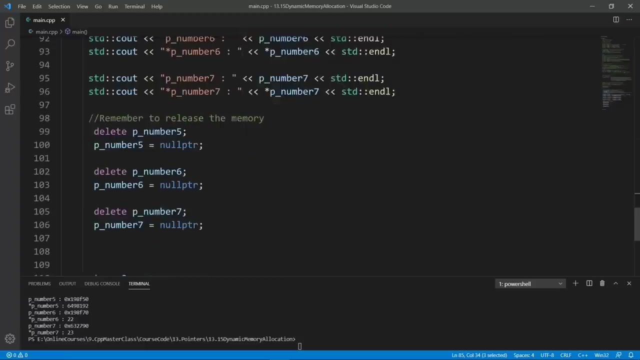 we have put that n at initialization here. the same is true for p, number seven. it's going to point to some address and we're going to have 23 and because we put in our 23, this is how you really use these pointers. another thing i want you to know is that, even if we have called delete and reset these pointers, 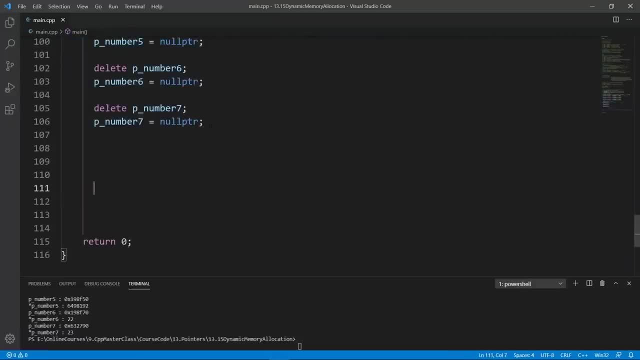 they are still available for use in our program. so if we want, we can reuse these pointers. so, for example, p number five, we can take it and use it to allocate new memory. so we can say new and and store in 81- why not? okay, so we can go down here and use that. this is going to be valid c plus plus code. 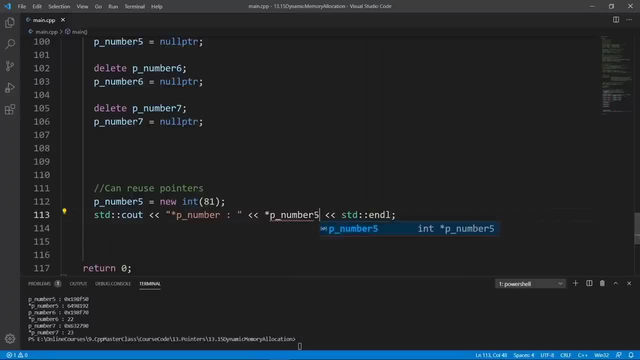 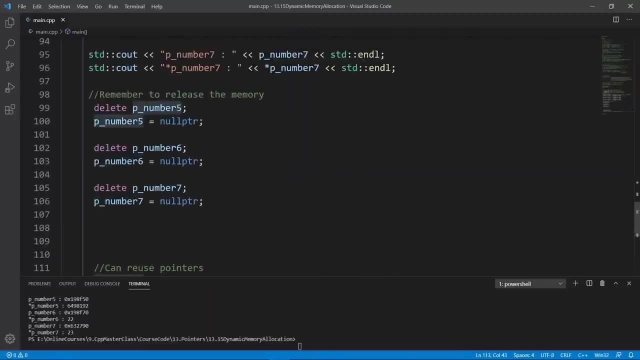 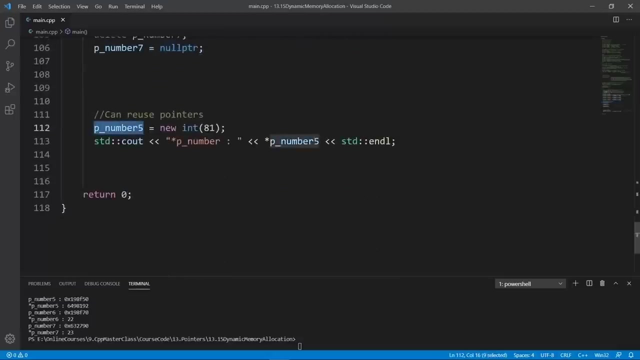 okay, take a moment and look at it. it is p number five, not p number, and official studio code is going to take this because it is valid c plus plus code. the memory has been returned to the operating system and the pointer has been reset to no ptr, but we can reuse the same pointer to. 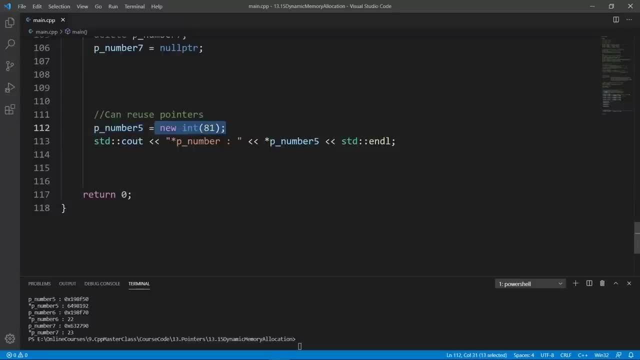 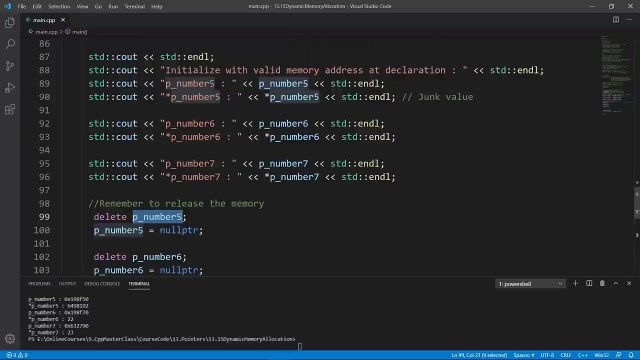 allocate new memory. so we are allocating new memory on the heap. the memory is going to be four bytes because it is going to contain an integer and we are using this pointer to point to that new memory. so this pointer is being reused. it was pointing to the memory that we allocated here, which was: 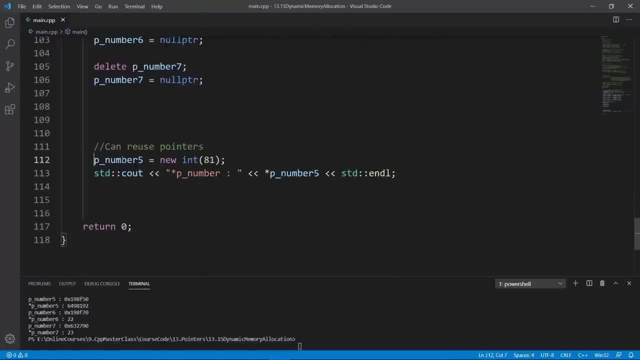 uninitialized and we are using that to point to new memory location on the heap. i really want you to understand these things because many beginners get them wrong and it is hard to correct these things in your mind once you have a wrong idea idea about them in the first place. so make sure you understand this. so if we print this, we're 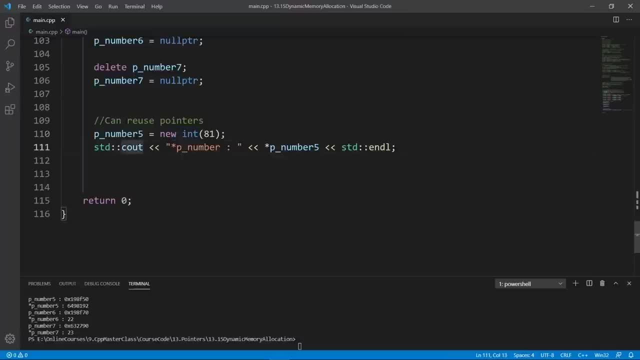 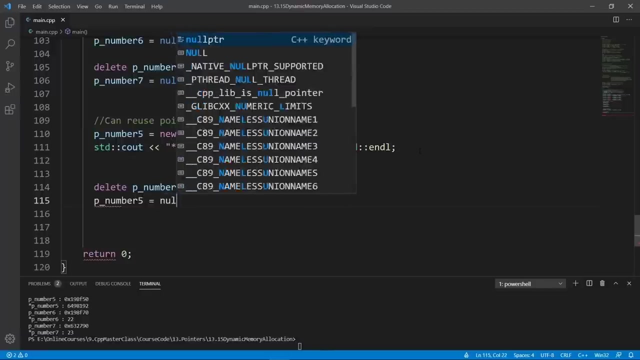 going to get the 81 printed out, but we have allocated new memory. we have to remember to release it again. so we have to come and say, delete p, number five, and we need to reset it to no pointer. and we're going to do that right here. once we do this, we're going to be playing it safe. let's try. 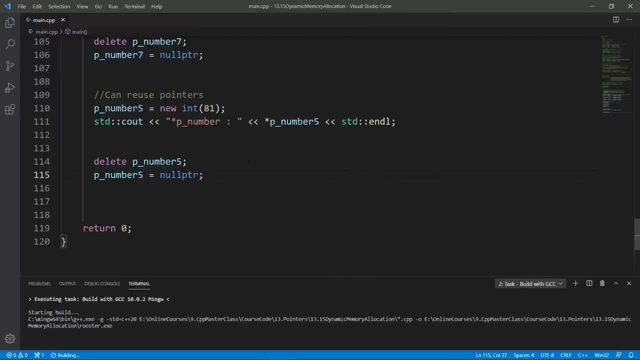 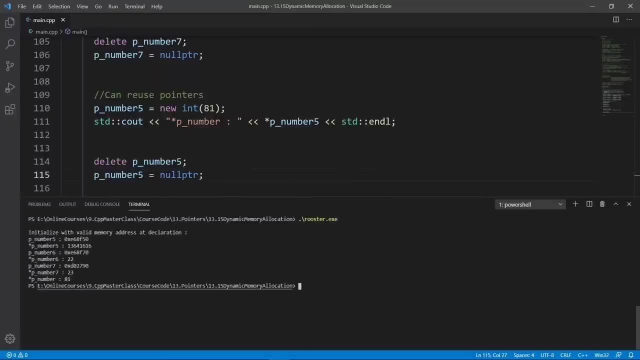 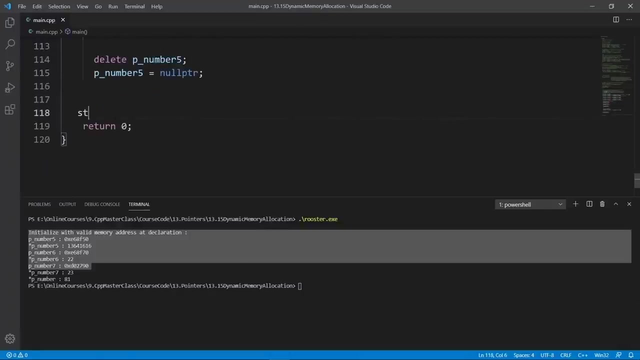 and run and see that we see the 81 printed out. we're going to build with gcc- the world is going to go through and we are going to clear and run rooster- and you see that we see our 81 and we don't have any crazy crash, for example. to prove that we don't have a crash, we can say that our 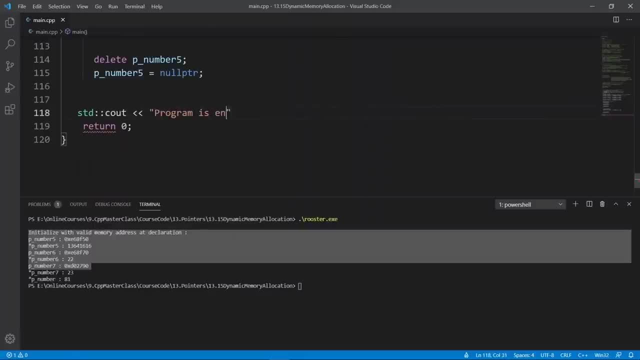 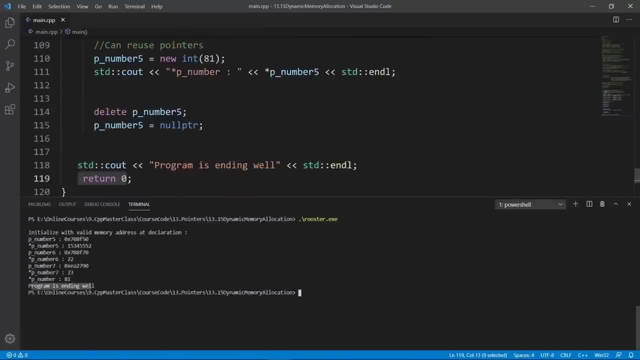 program is ending well, is ending well and we like to know if the program has actually reached the end before you. you it dies. we're going to build again with gcc and we're going to clear and run rooster and you're going to see that the program is ending well. the other thing i want you 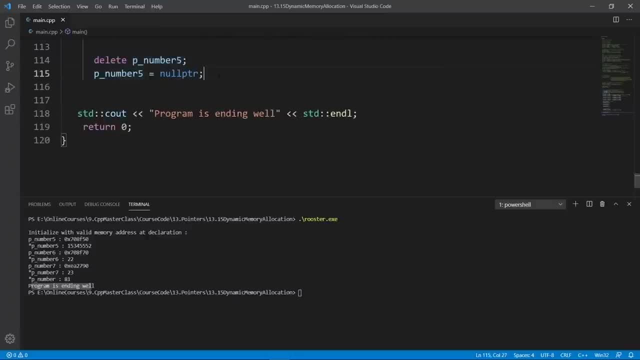 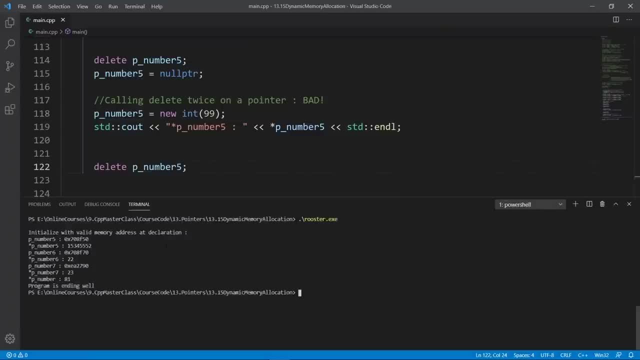 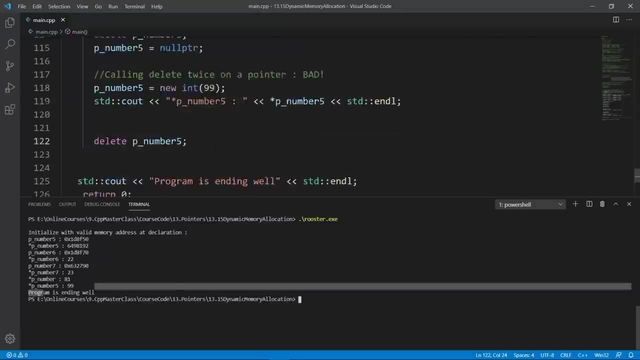 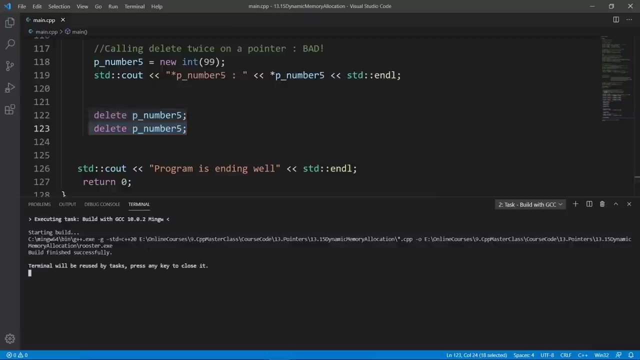 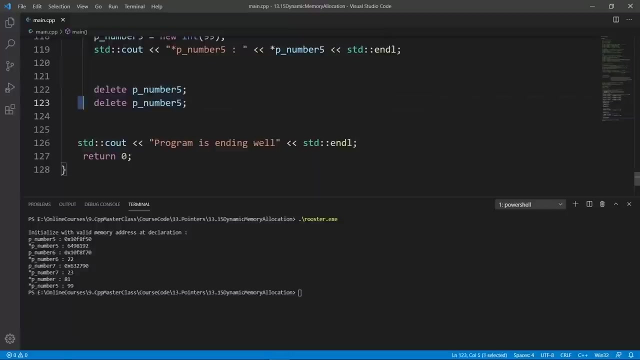 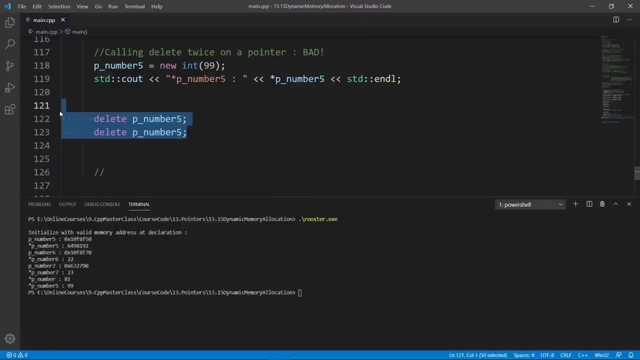 an example of that here. so we're going to see an example of that here. so we're going to see just a- so watch out for these kinds of things- and we're going to see different ways you can use to really make sure you are doing things right in c++. this is really all we set out to. 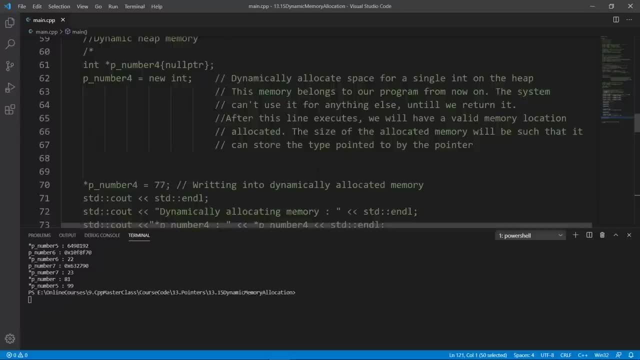 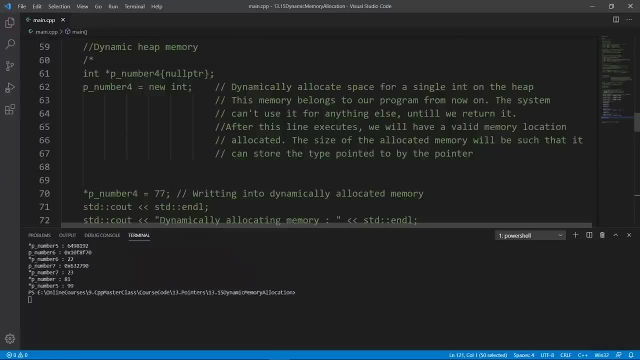 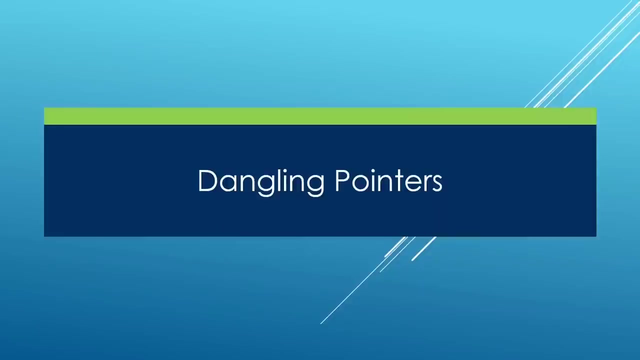 do in this lecture, giving you first-hand practice on how to do dynamic memory allocation. i hope you found this useful. we are going to stop here in this lecture and the next one we're going to learn about dangling pointers. go ahead and finish up here and meet me there. in this lecture, we're going 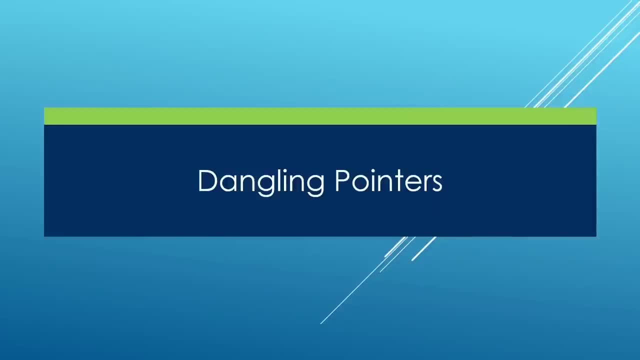 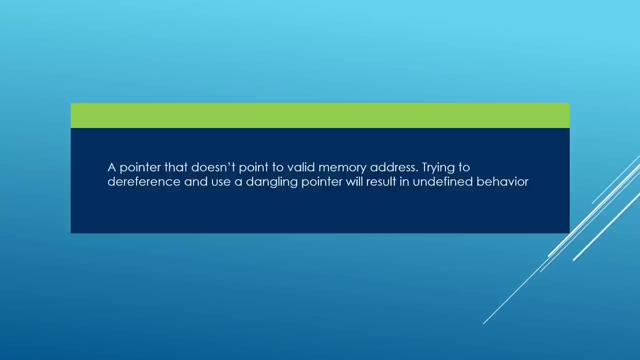 to focus on dangling pointers and show you how they can be bad. a dangling pointer is a pointer that is pointing to a valid address, and we have seen a few examples of this already, but in this lecture we're going to focus on that and show you common solutions we can apply to these problems. 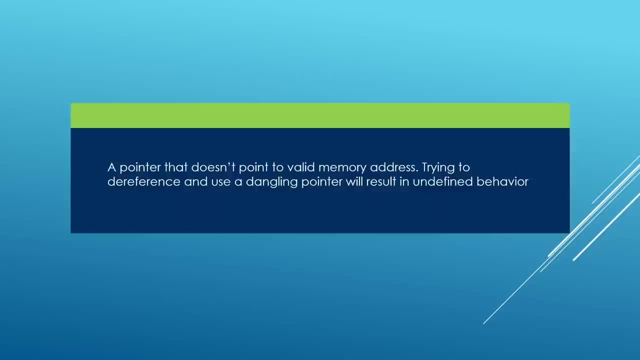 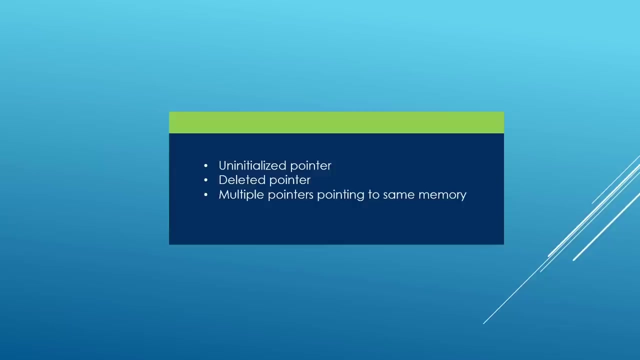 here and dangling pointers are really bad. they are going to lead your programs to undefined behavior and we have seen that that can crush your program many times. there are three kinds of dangling pointers we're going to look at in this lecture. the first one is a pointer that is not initialized. 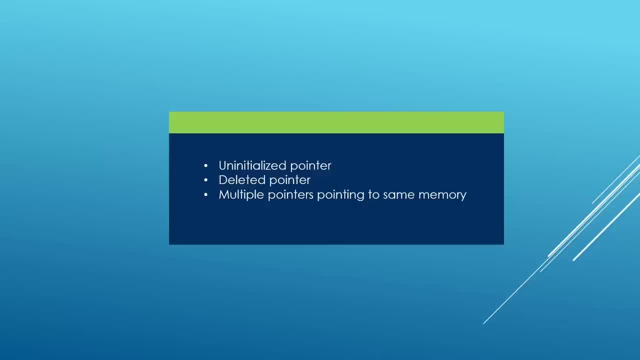 the second one is a deleted pointer. and the third case may come if you have multiple pointers pointing to the same memory location. and let's look at these cases one by one, one by one. here we have an example of a pointer that is not properly initialized. this is p number. 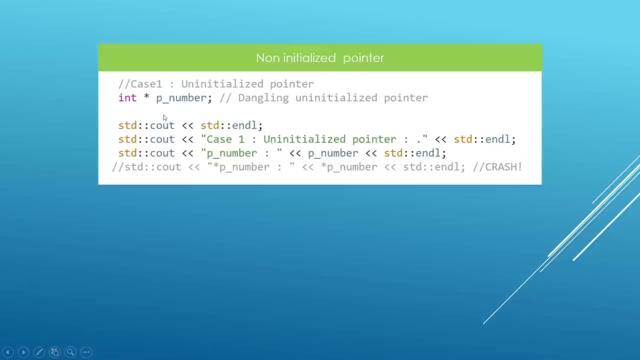 five, it is a pointer to end and it is not initialized, doesn't really point anywhere and it is going to contain junk address. if we try to dereference it, we're going to get bad things to happen because we don't really know which address is stored in there and putting something in there. 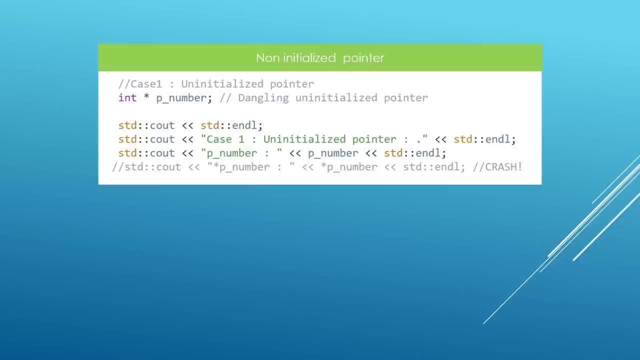 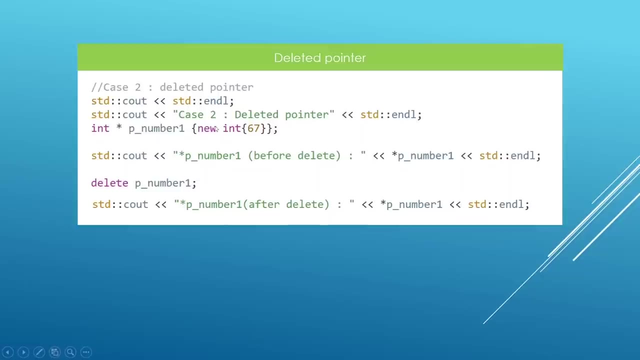 might lead to a crash. so this is something you need to watch out for. the second kind of dangling pointer that can really lead to a crash is a pointer that is not properly initialized. it doesn't really lead you to bad places- is a deleted pointer. here is a pointer p, number one. it is initialized with dynamic memory and 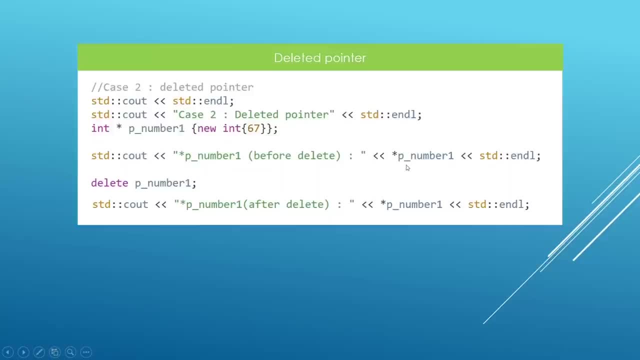 we can use it. for example, here we are: the referencing the pointer and printing the value inside and deleting the pointer. after we delete the pointer, don't really use it before you properly initialize it with some kind of memory. if we try to do that, this is going to be undefined behavior. and your program might crash. so make sure to deal with your program to get rid of the bit which doesn't delet it. enter the pointer p, number one, and shell it in something like this: warp it, because first program will always run out in the20 globally😏wicom. but you told me there's a bunch of zoom crews around you and you end up pursue pointing to duct tape or sitting there or on another device in the board, gathering this. 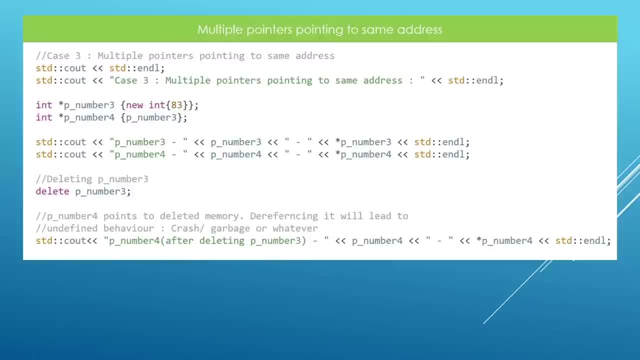 sure you don't do something like this in other cases. if you have multiple pointers pointing to the same address- and here is a simple example to drive the point home- we have pointer 3, which is pointing to dynamic memory. here we are using new ant in our braced initializer and we are putting 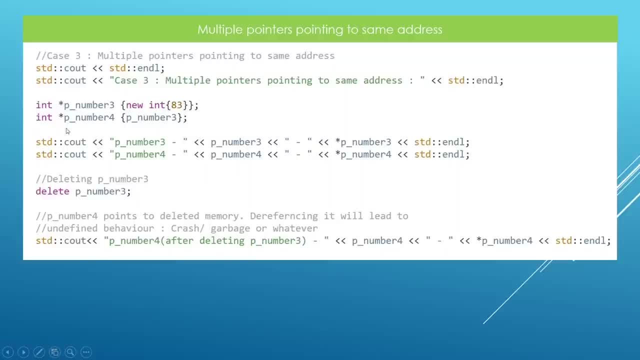 value 83 in that pointer location. and here we set up another pointer, p number 4, and we initialize that with another pointer and if we print these things out we're going to get that they contain the same address and they contain the same value. we're going to see that if we delete p number 3, 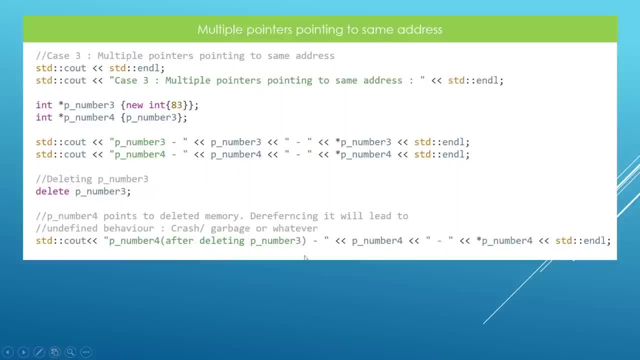 and try to use p number 4 later, we're going to get problems because this memory has been deleted by p number 3, but p number 4 is still pointing to that and if it tries to use that it's going to be deleted memory basically, and we're going to get undefined behavior. so be sure. 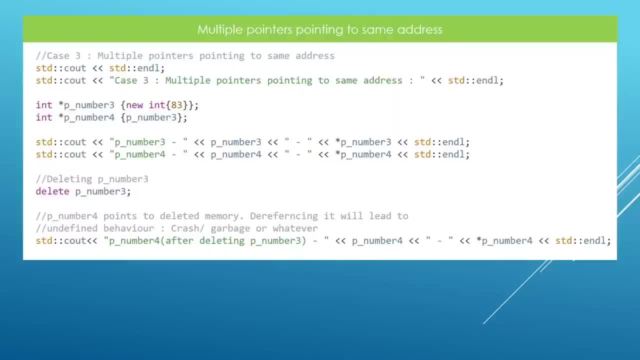 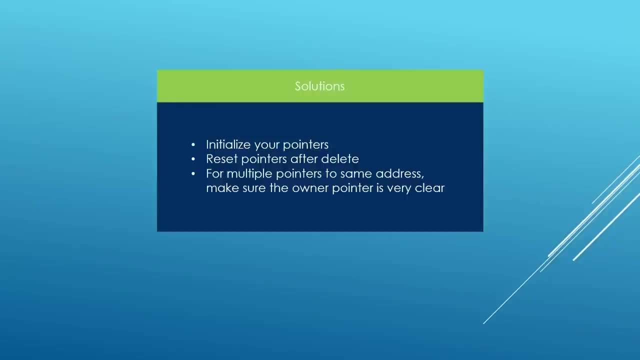 you know that you're not going to get undefined behavior, these problems, and try to avoid them in your programs. okay, these are problems, but how do we solve them? well, there are a few solutions. one is to always initialize your pointers. the moment you declare a pointer, make sure it is initialized. if you don't know what, you can initialize that. 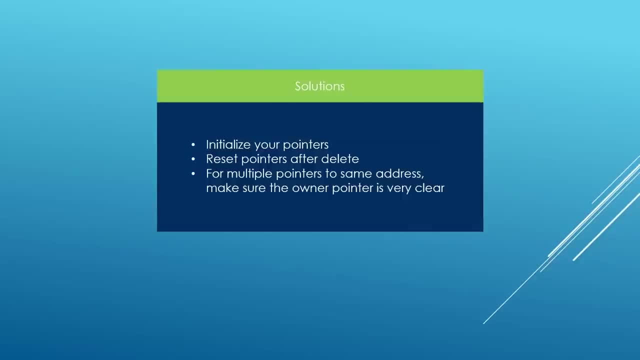 pointer with put in null pointer first and then you're going to put in an address later when you have a clear idea of which address you can store in. the second solution is to reset your pointers to the address you want to store in the address you want to store in the address you want to store. 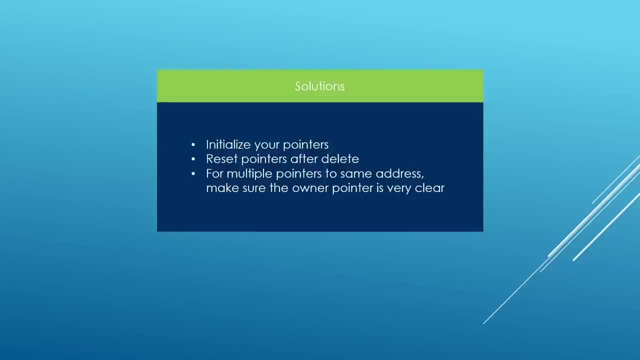 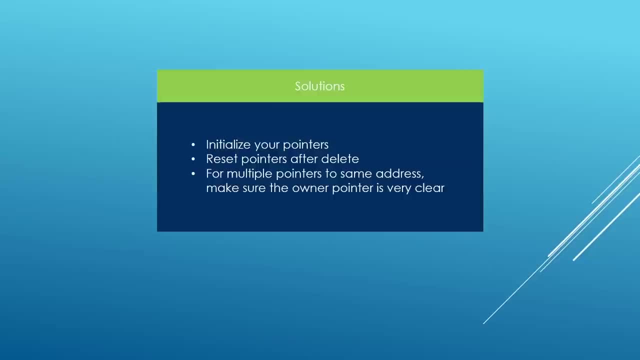 memory location contains a valid address. before you do that, and for multiple pointers pointing to the same address, you have to choose and make one pointer, the master of the controller of the memory. and all pointers are basically going to be slaves which can't release the memory, but they can read and do something with that memory, but they don't. 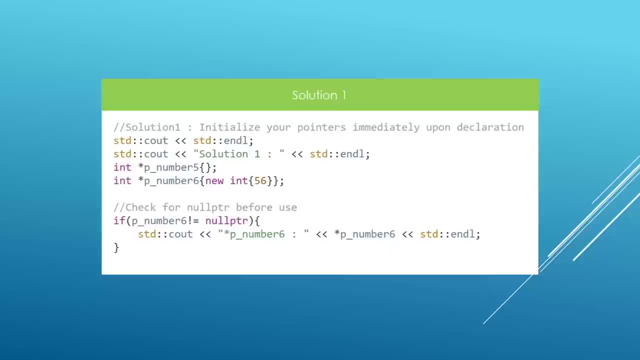 have the task of releasing that memory, and here is how you can apply solution one. for example, we have pointer number five and we're going to brace initialize it. this is going to initialize it to null pointer. the other thing you can do is initialize the pointer with dynamic memory, like 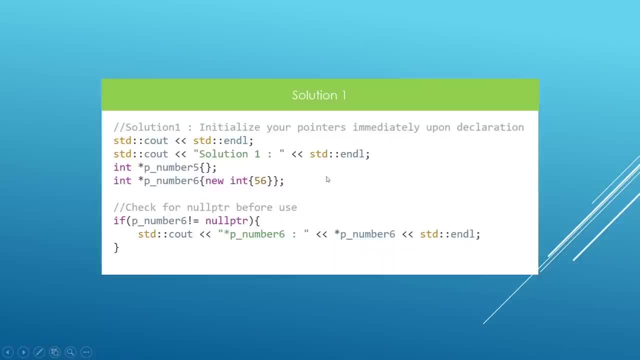 we are doing here with p, number six and this is going to put in the value and we are going to be playing on the safe side. now, if your pointers are initialized, developers have a chance to check your pointers against null ptr to see that they contain something valid before they use it. and if they see that, 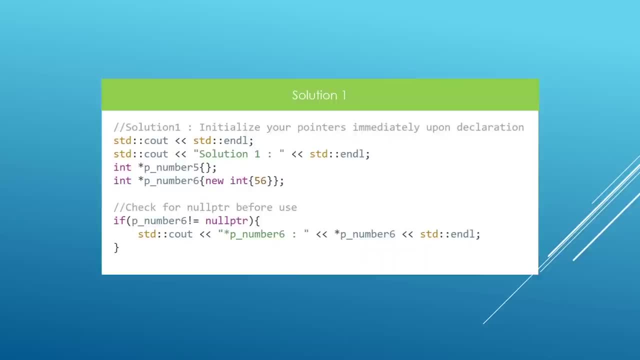 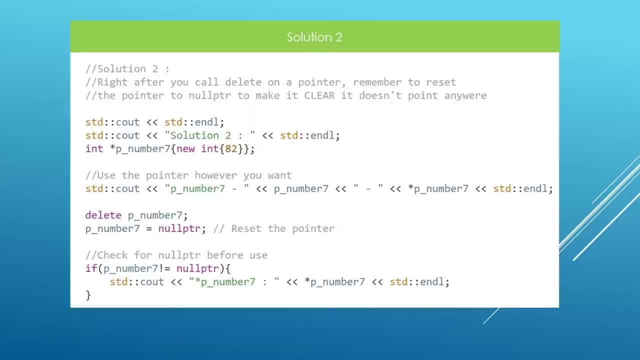 it contains null ptr, they are not going to try and use it and this is going to be very safe. for the second problem with deleted pointers, we are going to reset our pointers after we call delete. for example, here we have p number seven initialized with dynamic memory, and. 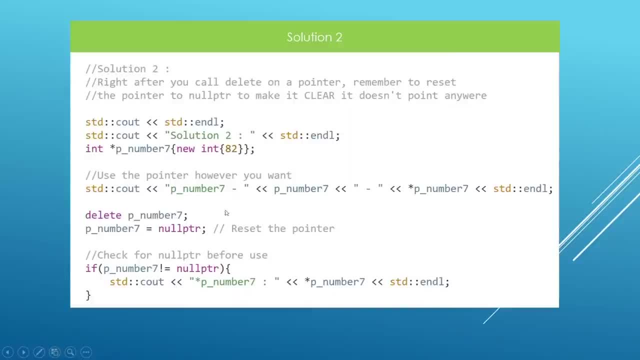 this implies that we can go ahead and delete these same pointers that we were using and clickanie to преп it and set various parameters to our new pointer. so do the same thing i do. we don't apply element wasp or our危 edition function and then we just select nonnullptr. 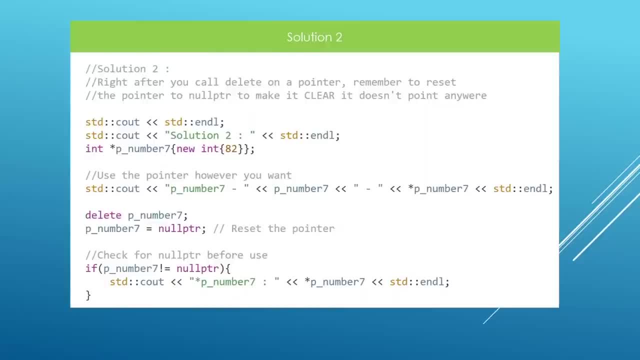 so that other developers or even ourselves can check this memory against nonnullptr and if it's different from nine ptr, we can use it. if it's equal to no ptr, we're going to leave it alone and do something else. this is going to be very safe if you have multiple pointers pointing. 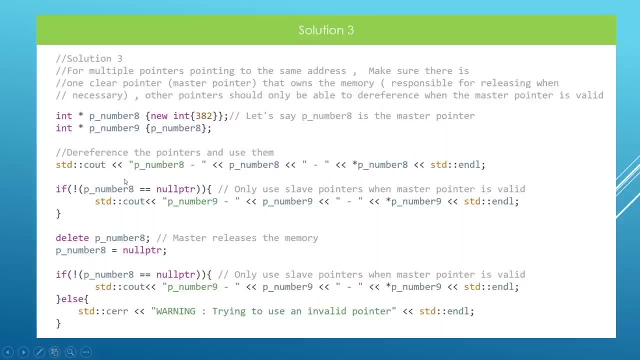 to the same address, like we have here. then you're going to have to decide which pointer is the master pointer and other pointers are going to be slave pointers. and before use, all the other pointers are going to check against the master pointer and see that it contains valid memory, because the master 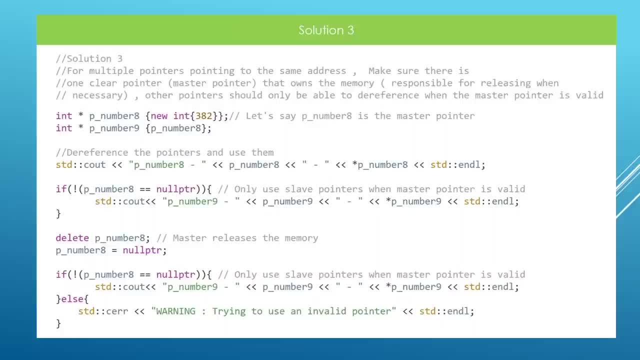 pointer has the task of deleting this memory. let's go through this and see how this could work in practice. so p number five is our master pointer. we are setting p number five and initializing it with p number eight. we are creating things using p number eight. we can either use p number eight or 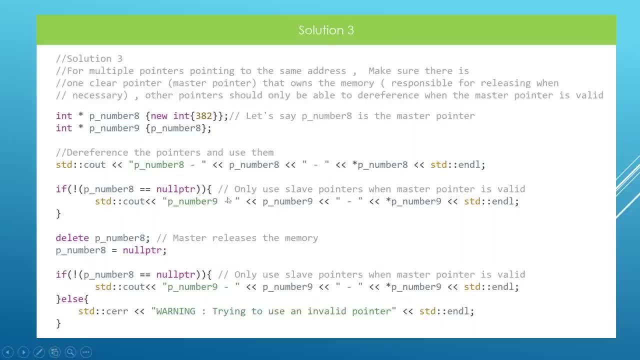 p, number nine. this is going to work. but before we use the memory location, we're going to check against the master pointer. if the master pointer contains null ptr, we're not going to use this memory. if the master pointer doesn't contain null ptr, we're going to use this memory here. okay, if? 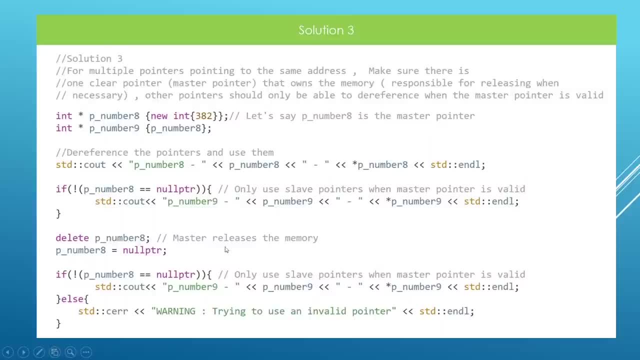 you go down, you see that the master pointer is going to be releasing the memory and if we try to use that memory after it was deleted, we're going to see that it contains null ptr and we're not going to be using it. this is something cool and it is really easy to implement this safety guidelines in your programs now that you. 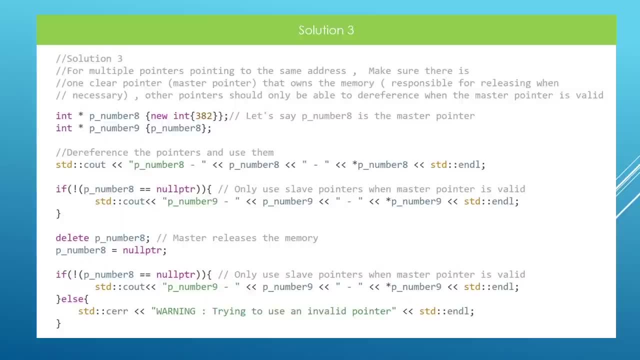 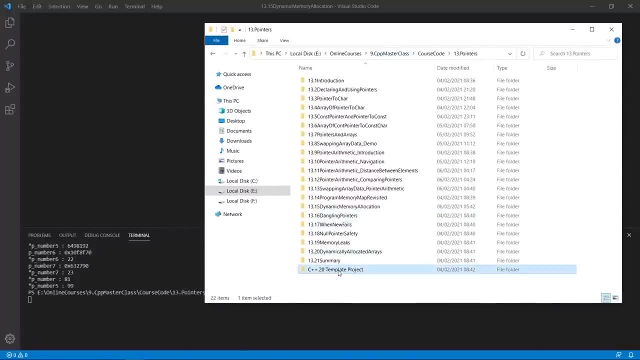 know about this. we're going to go to visual studio code and show you this in action. okay, here we are in our working directory. the current project is dangling pointers, so we're going to grab our template files pretty quick and put that in our project and we're going to open this in visual 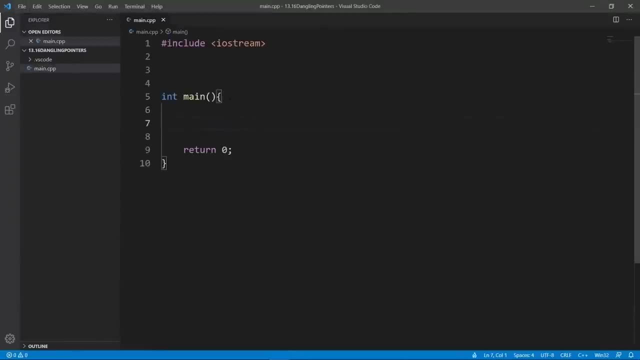 studio code. we are going to look at the first case of a dangling pointer, and this is a pointer that is not initialized properly like p number. here, if we try to dereference it, we're going to get something bad to happen. so let's see that and let's go down and say that program is ending well, just to know that. 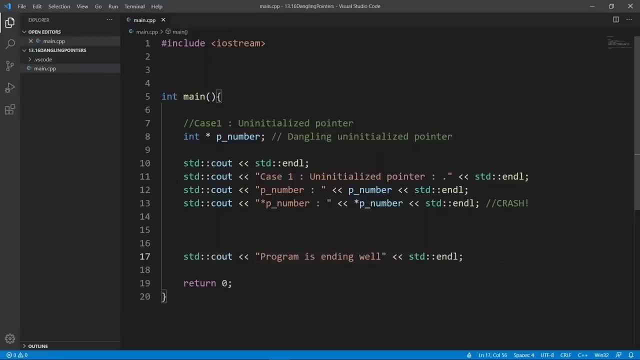 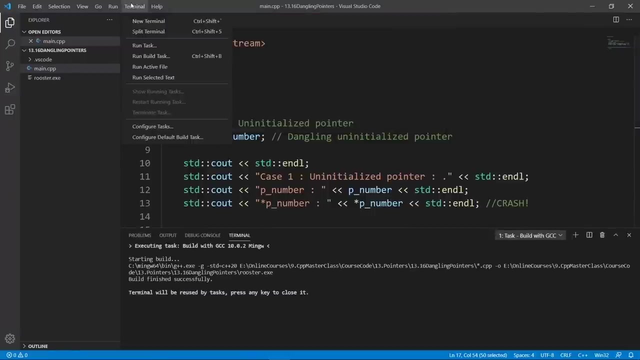 we didn't get a crash, because a crash is basically going to terminate your program on the offending line. that's what it's going to do. so if the program works well and ends well, we're going to print this line here. let's bring in gcc to weld this program and let's open a terminal so that we 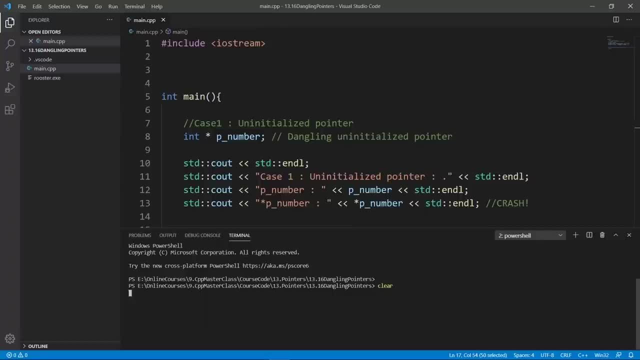 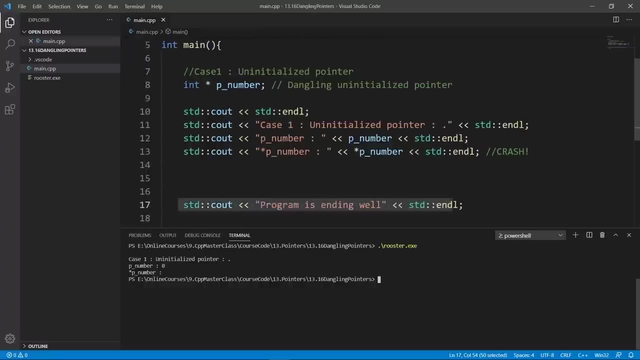 can run it. we're going to clear the world was good and we're going to run rooster. you see that the program didn't end well. it crashed. and it crashed because we are trying to use uninitialized memory when the operating system is going to try and run this thing. it's going to see. 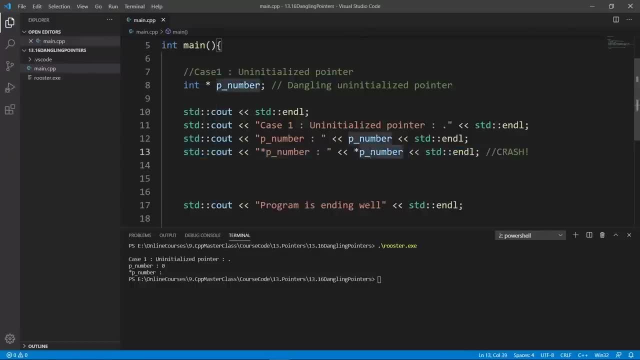 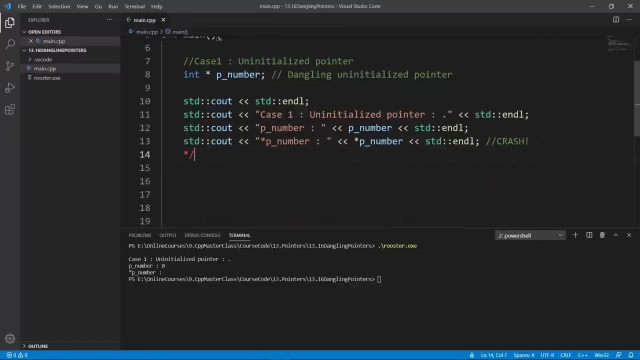 ah, this guy is trying to modify memory that doesn't really belong to him. it is a rogue program. i am going to kill it and it is going to be terminated on this line here. this is really bad. you should avoid these kinds of situations, so don't do this. we are going to comment this out and show you another offending thing we can do. 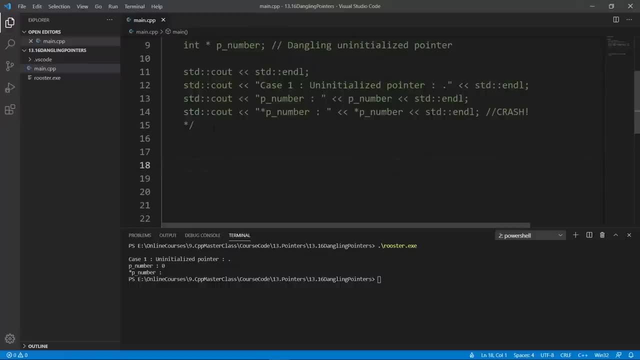 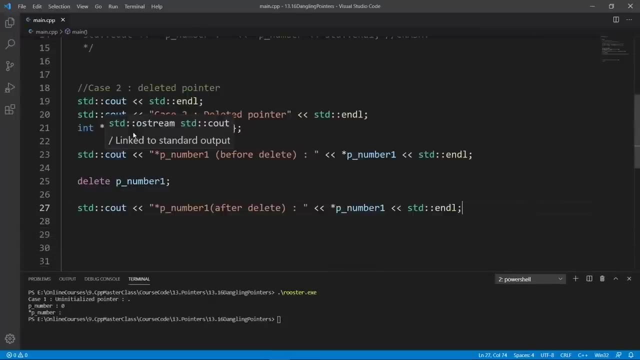 in our program and that is using a deleted pointer. if you do that, you're going to get something bad in your programs. so here we have a small example. we have a pointer to end, we initialize this with a dynamic piece of memory and we're going to store in a 67 and we can print this out. this is going to: 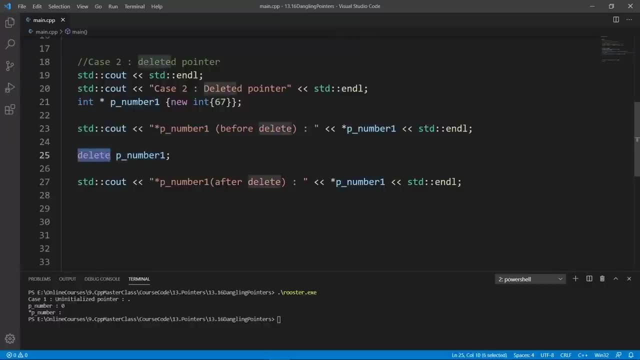 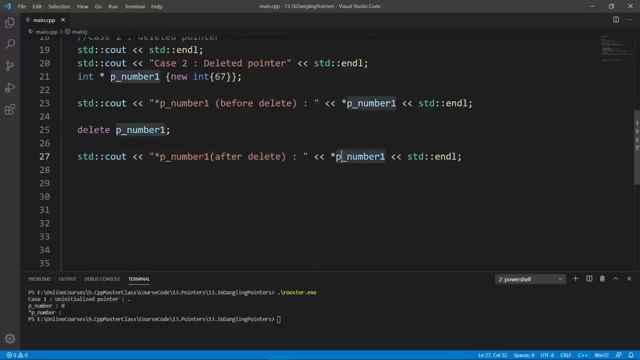 work pretty well, but we delete the memory down here and we try to use it after we have deleted the memory. so the operating system is not going to be happy about this, because once the memory is deleted it is no longer our memory. so we have no business dereferencing pointer one and trying to 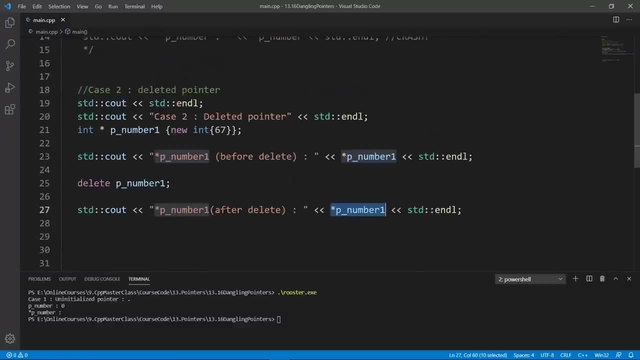 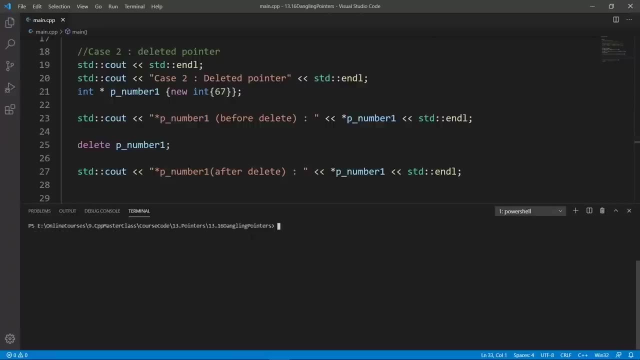 use that here and we're going to get a crash and this is something you should avoid. so let's try and world this and show you this in action. we are going to clear and run rooster and you're going to see that program is ending well, but in some cases it might crash and hopefully 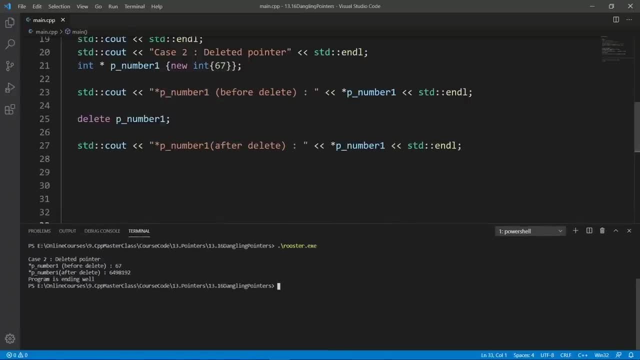 this shows you the danger that this things might put you into. sometimes your program is going to seem working fine, but sometimes, when this memory that we are pointing to in p number one here, is being used to do something really important to you. so let's try and world this and show you. 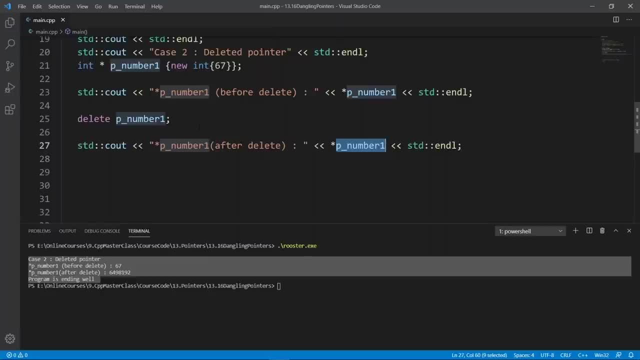 that this is going to crash and we're going to delete the memory and we're going to use it after we have deleted the memory and we're going to see that this is going to crash and we're going to see that this is going to be. 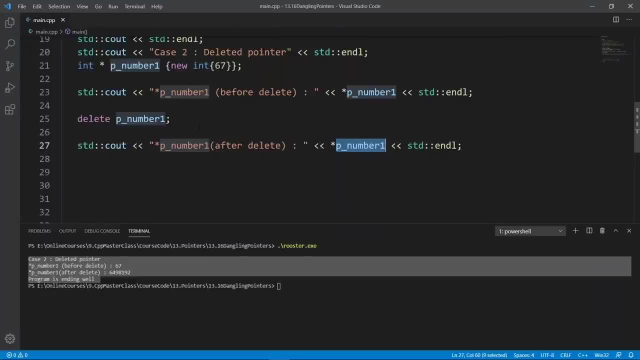 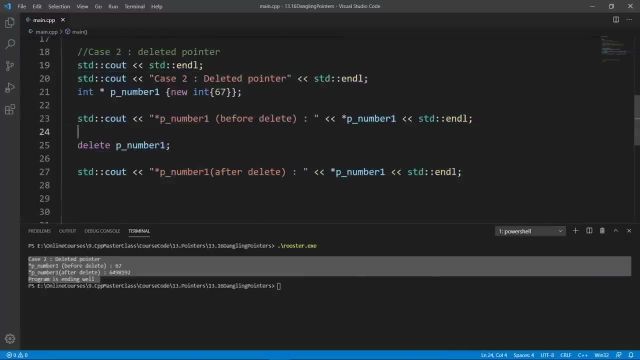 the same behavior every time you run your program. some of you might be saying, uh-huh, the program is working here. daniel, why are you making this such a big deal? well, it is a big deal because you are not guaranteed to get the same results every time you run this program, so be sure you really avoid. 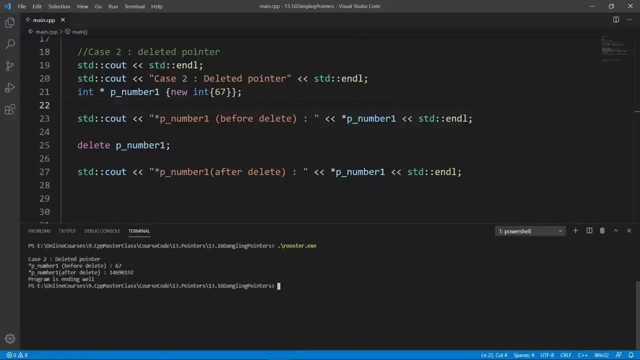 these kinds of situations. let's try and clear and run the program again. hopefully we're going to see it crash, but we're not okay. so let's clear and rebuild again and see that we have a better luck that time. let's clear and run rooster. it is going to end well, but you notice that we are trying to. 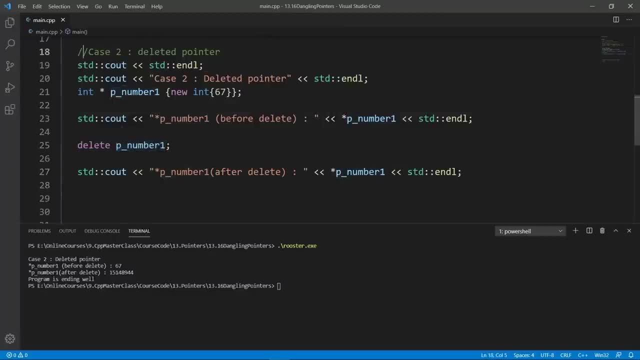 use a piece of memory that has already been deleted, and this is bad. don't do this. make sure you don't do something like this. we're going to comment this out again and show you another offending thing. we can do with our programs and bad things might happen if you try to have multiple pointers pointing to the same address. 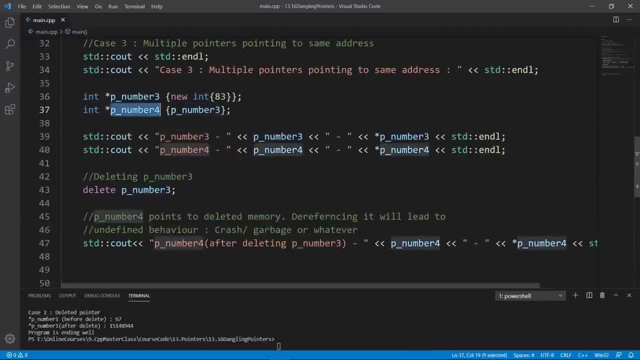 and that's what we have here. we have p number three and p number four here. p number three is allocating new space and it is pointing to it. we have an 83 inside and a p number four is initialized with p number three. we can do that, so these two pointers are basically pointing to the 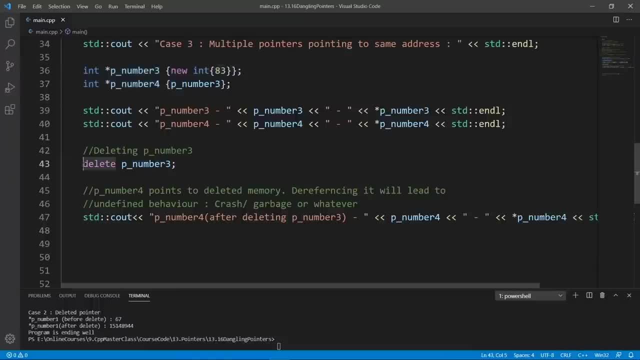 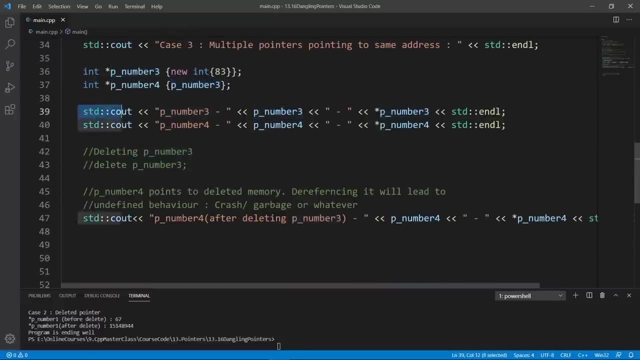 same memory location. let's run this and show you that we're going to comment out this, delete statement here and run the program first to really prove that they are pointing to the same addresses and they contain the same values. let's build and run- we're going. 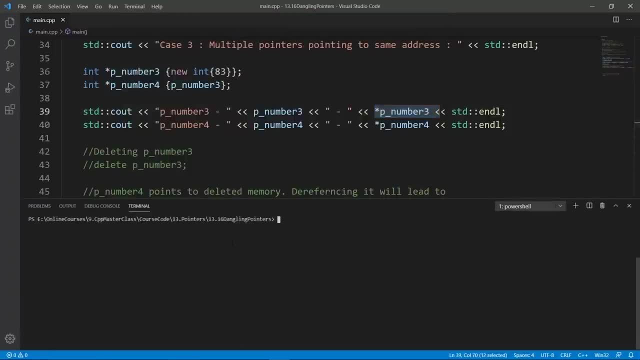 to use gcc for that and we're going to clear and run roaster and you see that p number three, the address is this and it contains an 83. p number four contains the same facts. so let's see what happens if we try to delete using p number four and p number five and p number five and p number. 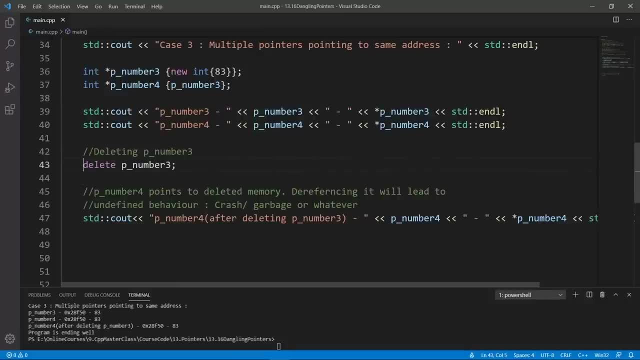 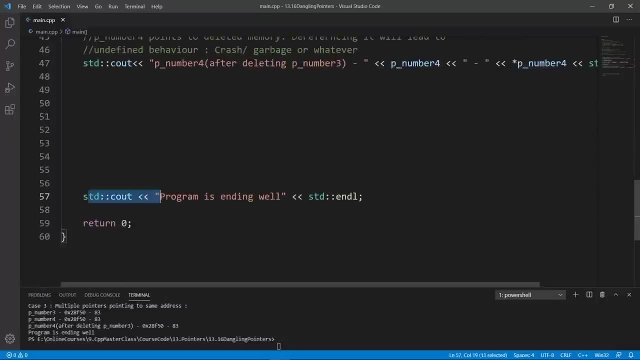 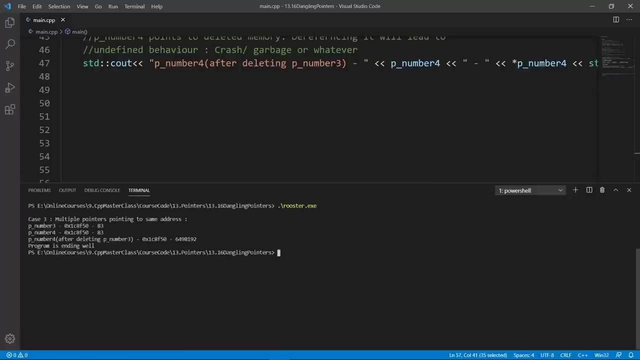 three and using p number four later to try and read stuff. this is what we are doing here and we're going to see if the program actually gets to end. well, we're going to weld again. the world is going to be good. let's bring this up and clear and run rooster and you're going. 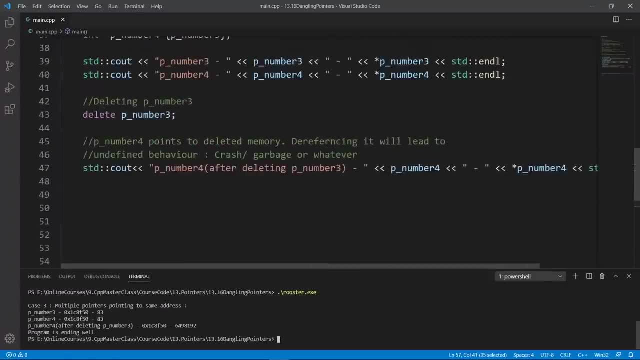 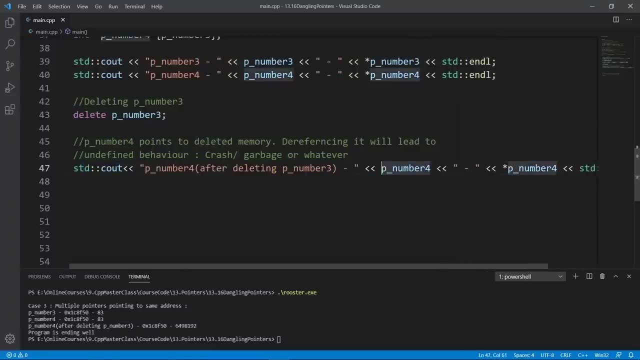 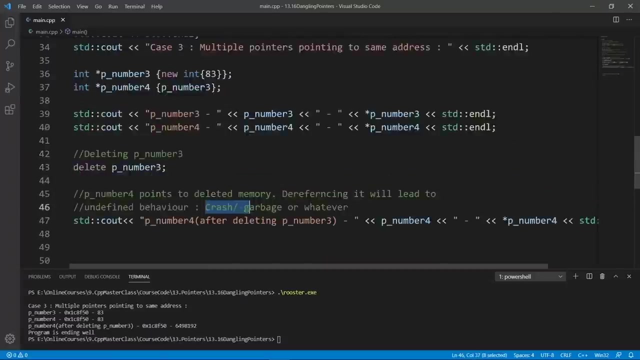 to see that the program is also going to end well, but we are using a deleted piece of memory here and anything can really happen, okay, so you might get garbage, you might have really any piece of junk inside, or you might get a crush in some extreme cases, so this is really bad. 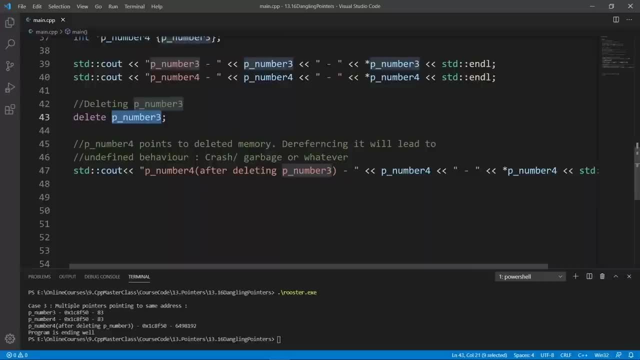 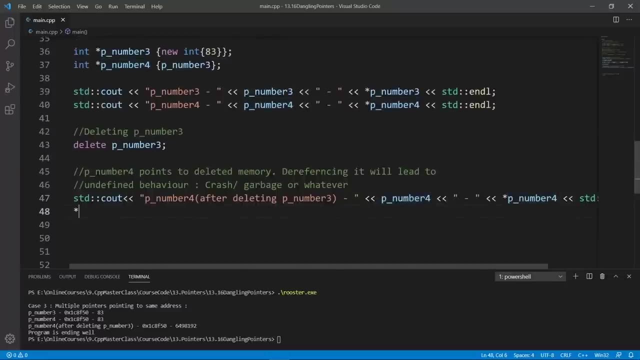 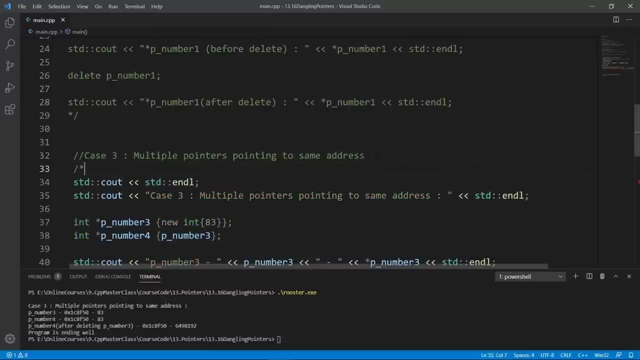 don't do it. don't try to use a piece of memory that you have already deleted through a pointer, and these are problems you might run into in your programs if you try to use dynamic memory allocation. let's look at how we can solve them, and the ultimate advice is to make sure you put 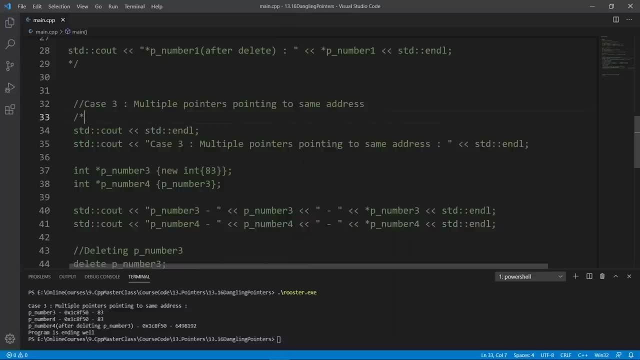 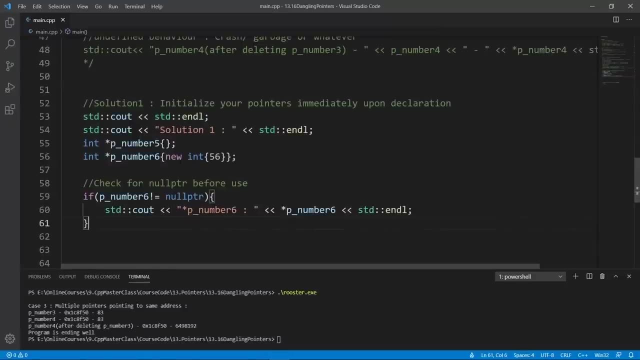 a null ptr in a pointer if you don't know what that pointer is actually storing. okay, let's go down and look at solution one. solution one is to initialize your pointer to null pointer. every time, if you don't have a value, you can put in use null ptr. that's what we are using here implicitly, but we can explicitly. 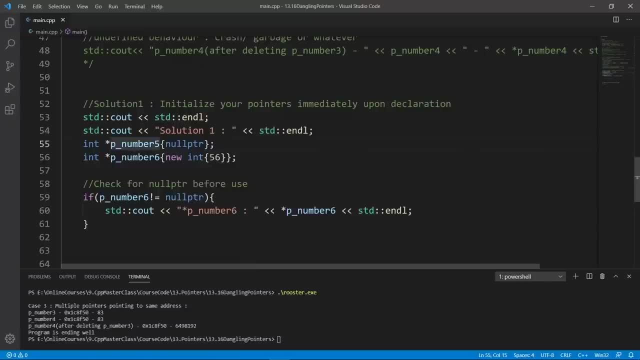 put that end because it is good. and before you use a pointer, you have to check and see if it doesn't contain no pointer. this is how we do it: if pointer 6 is different from no pointer, we're going to use it. if it is equal to no pointer, we're not going to use it, and we're. 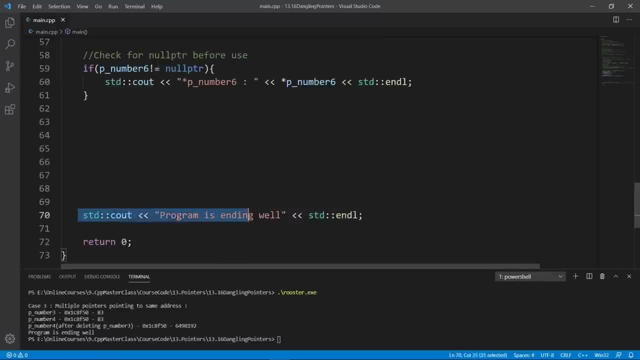 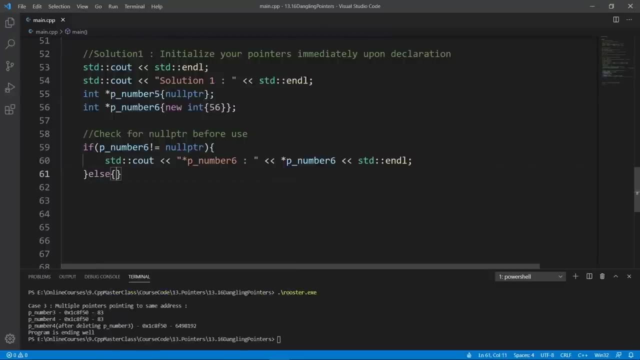 going to be playing on the safe side and you're going to see that the program is going to end well here. if we have a null ptr inside, we can say else here and say invalid address, okay, and that the user is going to know that they are trying to do something really bad. so let's try and check. 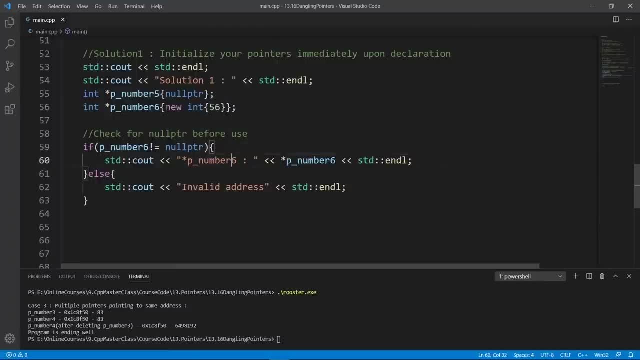 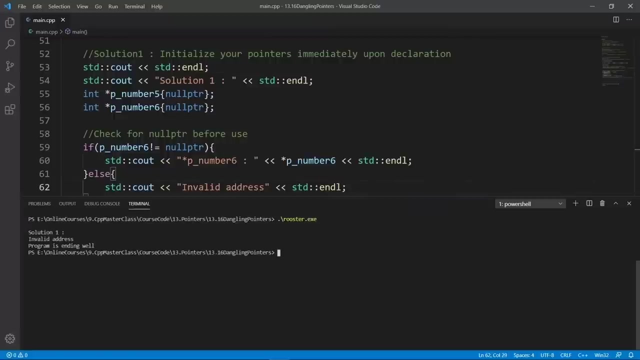 against p number five. so let's go and store a null pointer in p number six to really try this out and show you that we're going to get this warning. if we're trying to use it and we're going to build with gcc and we're going to clear and run rooster, you're going to see that invalid address. 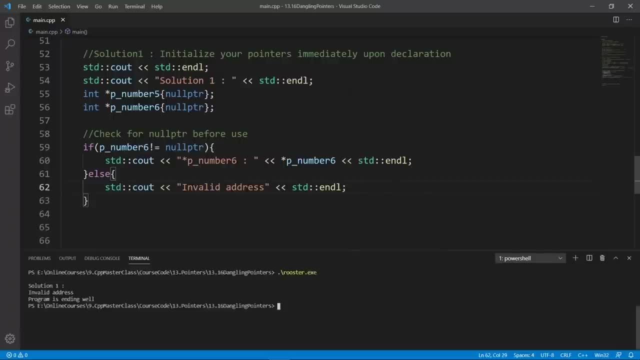 and the program is going to end well, and if we try to put this statement somewhere where we're not shaking against null pointer, we are going to get a crash. so let's comment this out so that it's clear what it is we are running here. so if we run this, we're going to get a crash. we have seen that, but let's show this again. 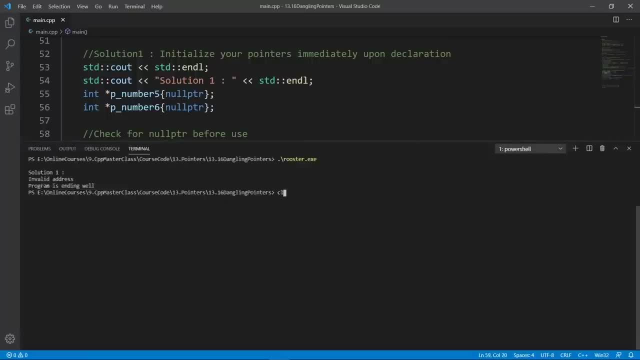 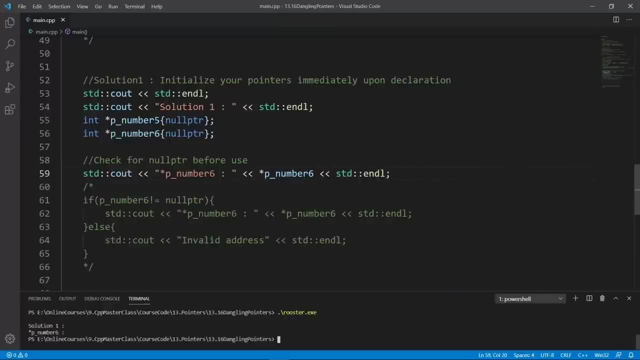 and really highlight that we are solving the problem here. if we run rooster, the program is going to crash because we are trying to use an initialized memory. but if we try and check against no ptr, like we are doing here, let's do that. we're going to be playing. 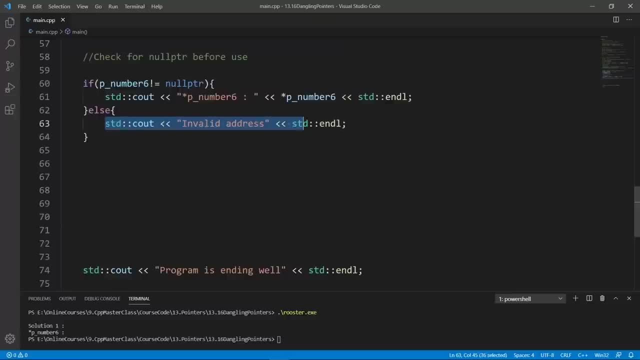 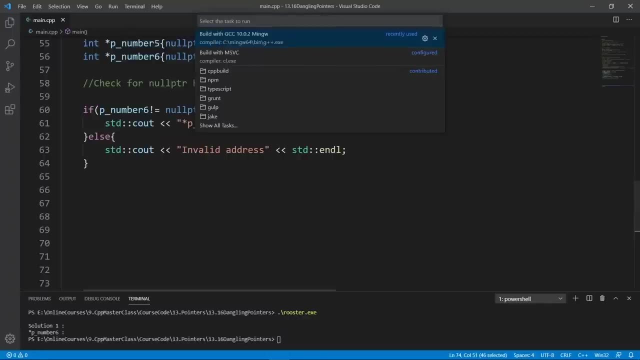 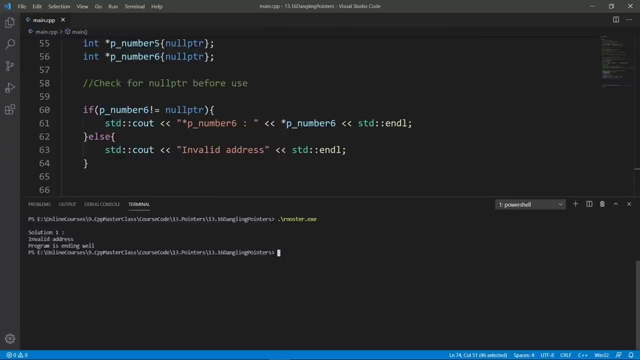 the safe side, because it's going to tell us invalid address and we're not going to get a crash and the program is going to end. well, this is really cool, so let's try and do that again. we're going to world, the world is going to be good, we can clear and run rooster and the program is going. 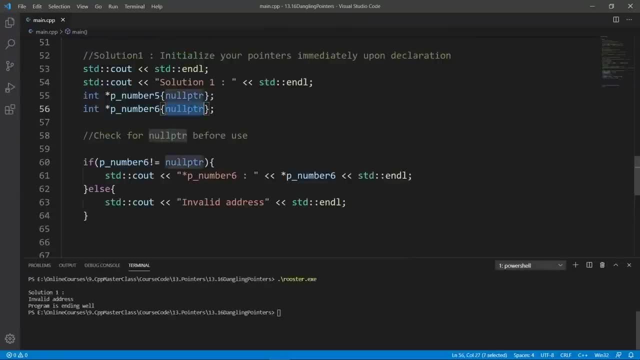 to end well, okay. so if we have a value inside, we're going to get that. so let's put that n and say new ant and put in an 87, for example. it doesn't really matter what we're putting, so we're going to build again. the world is going to be good and we can run rooster, and you see that. 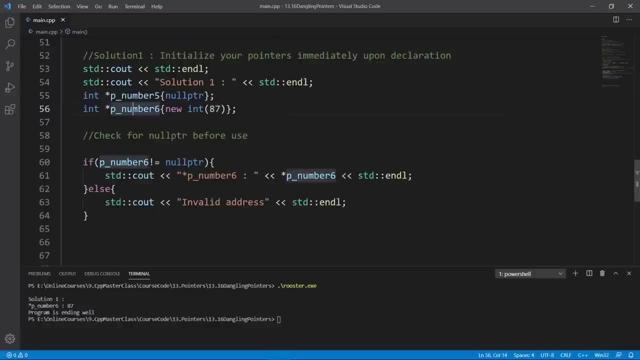 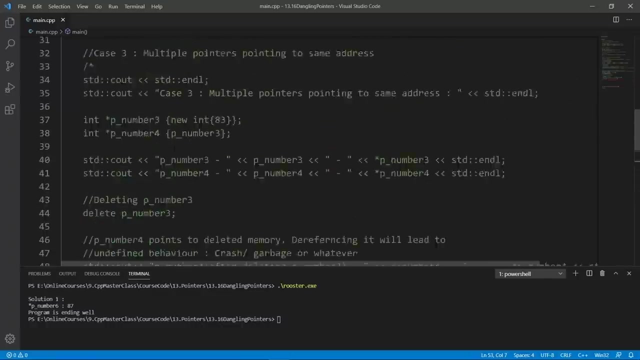 we are getting a value here if we are not storing null ptr in p number six, and you can do the same checks against p number five. but i think this is really enough. so this is one way you can avoid dangling pointers. the next thing we're going to look at is if we are using a deleted pointer. 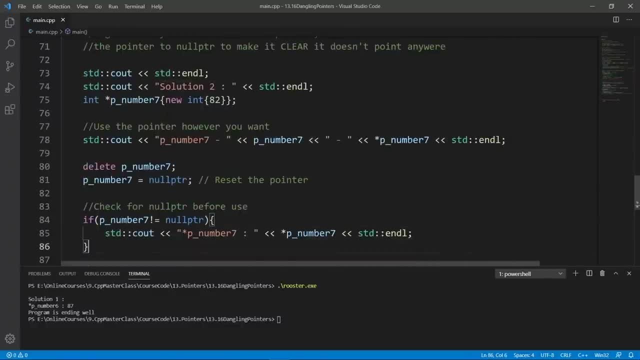 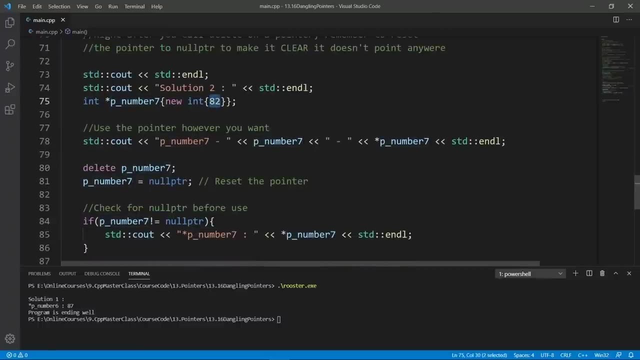 and again. the solution is to set a pointer to null ptr after we delete it. here we have p number seven. it has 82 inside. we are using it here and printing stuff out. we're going to delete it after we are done using it and after that, the first thing we do 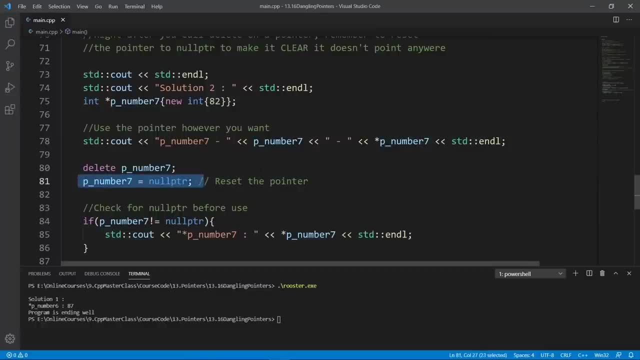 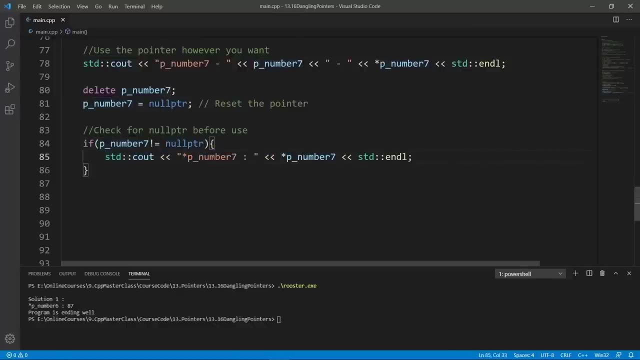 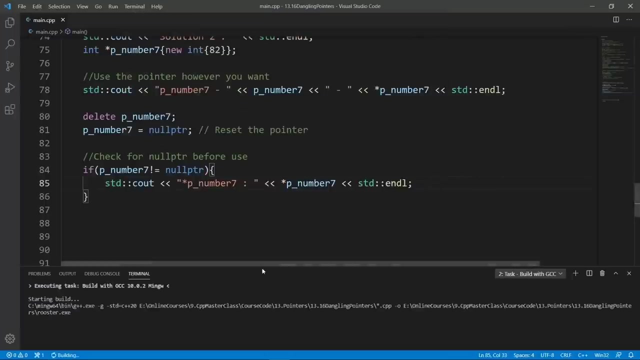 is to reset it to no ptr. when we do that, other people or even ourselves have a chance to check it against no ptr and we're going to know that it doesn't contain anything useful for our program. and if we do something like this, we're not going to run into all these weird problems and our program is going. 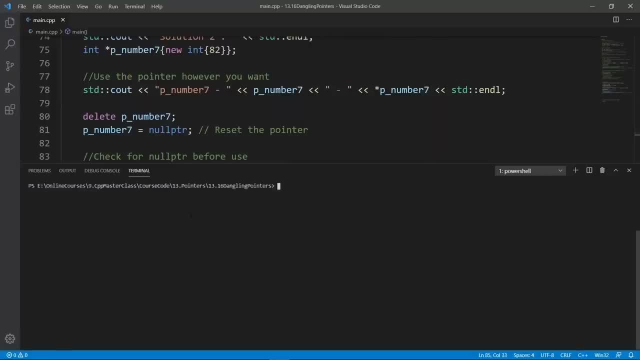 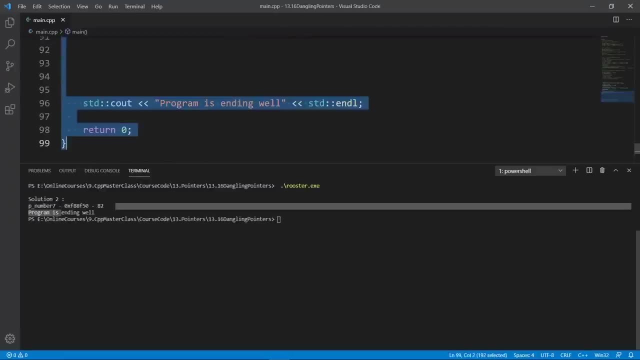 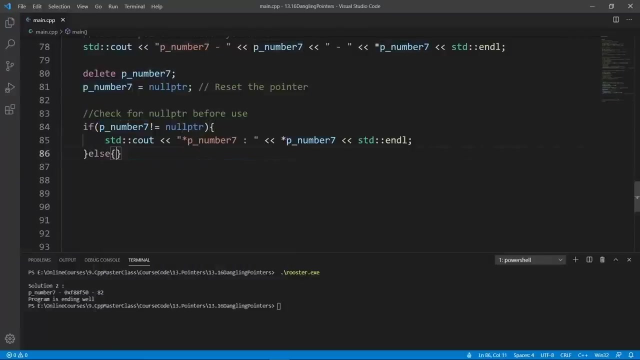 to have consistent behavior across different runs, and this is really cool. so we're going to run this, we're going to get things printed out and the program is going to end well, because right now we are checking against no ptr. we can even be explicit in showing the warning. here we 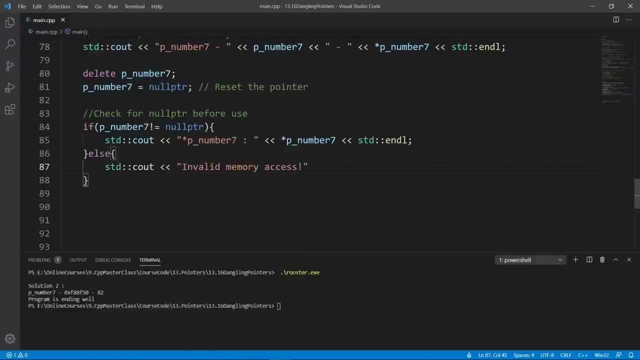 can say invalid memory access and if you run this program you're going to really know all your data runs in the question screen. we want to give us memory access. so maybe this is the problem here for this case. you know there are some things in there, but for this case we are your continued déplacement. 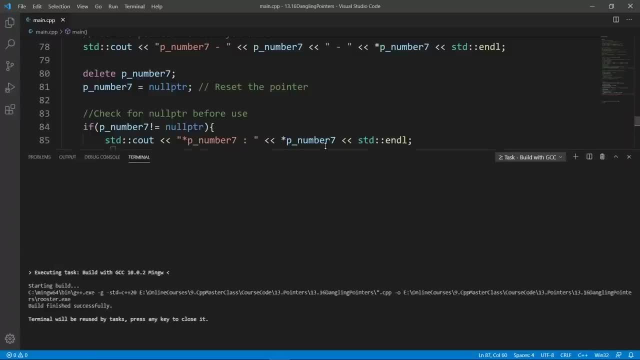 know this. so let's finish this up and we're going to bolt and the world is going to be good. if we run this and run rooster, we're going to know that we are doing an invalid memory access after we have deleted the pointer and this is going to save you from possible crashes that you might. 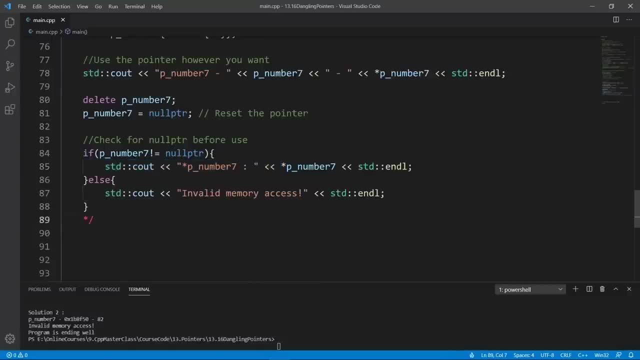 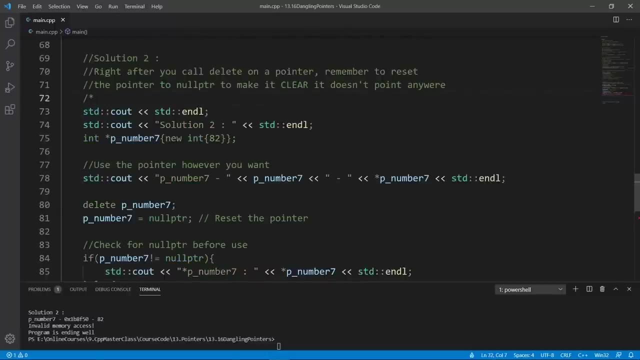 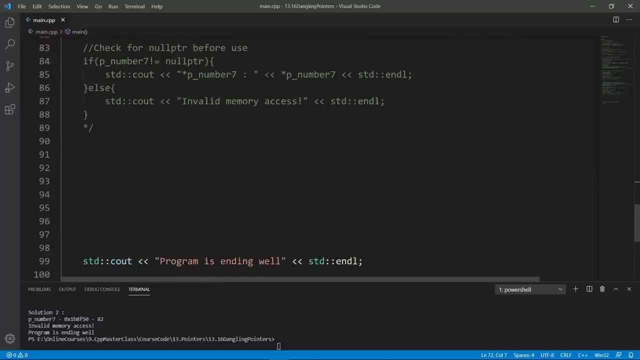 experience if you don't do this. so this is a second solution you might want to implement in your programs, and we're going to comment it out and show you how you can get away from the problem of when you have multiple pointers pointing to the same address. we are going to go down and put 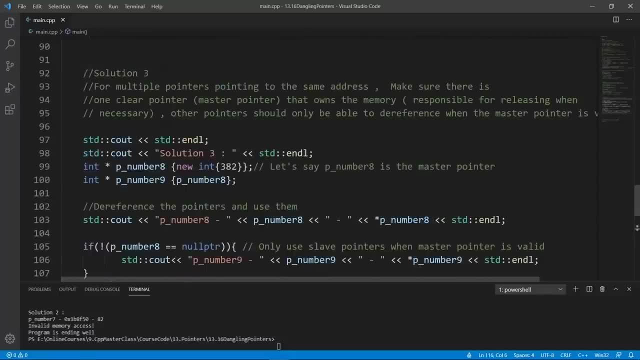 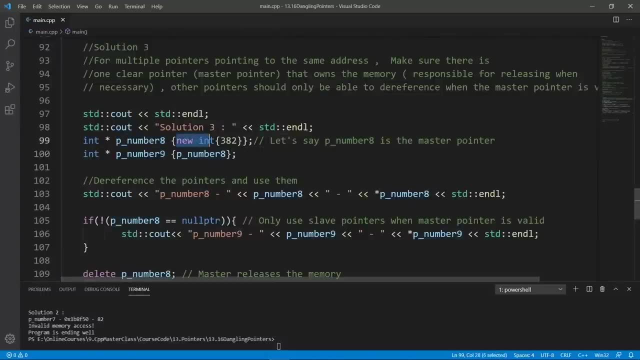 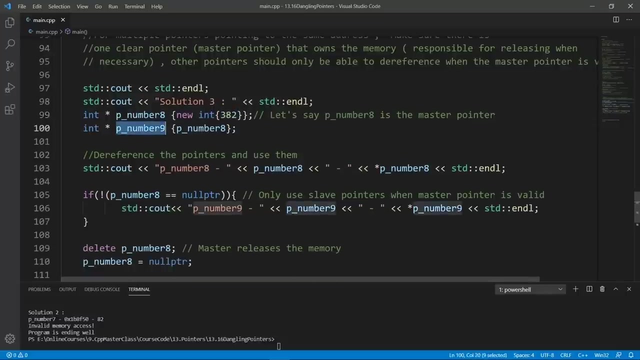 in the code. it is what you have seen in the slides and it is really nothing new. so we have pointer eight and pointer nine here and p number eight here is pointing to dynamic memory and the value inside is 382. p number nine is initialized with whatever we have in p number eight. so they are. 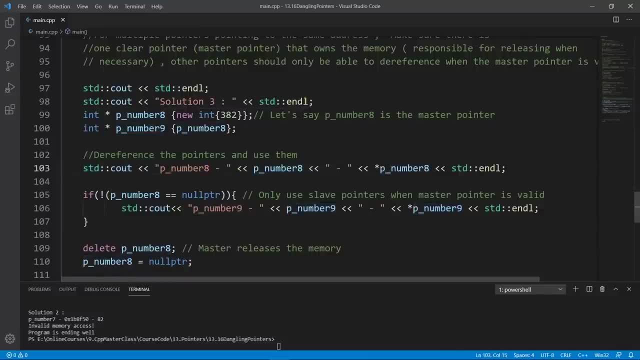 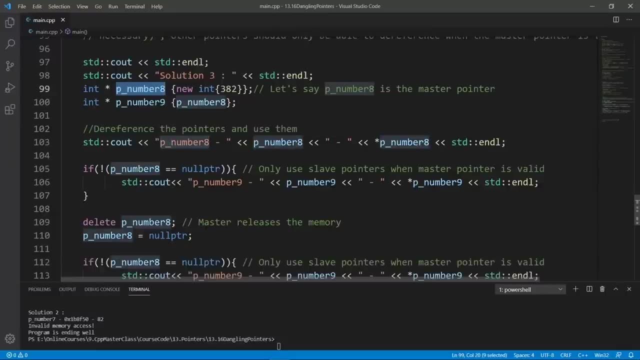 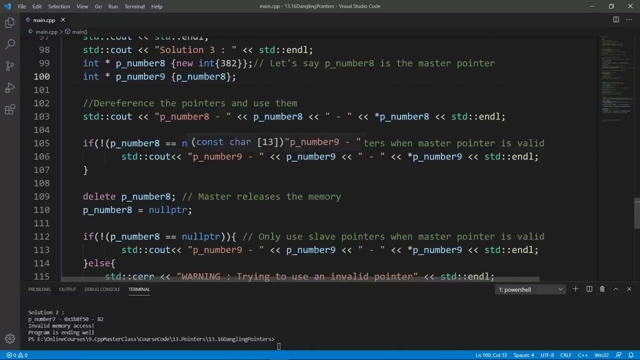 going to be pointing to the same addresses here, but we have made p number eight the master pointer, so it is the only pointer that is going to be able to delete this memory location, even if we have multiple pointers pointing to that. okay, so every time we want to use this memory, we have the option to check against the master pointer and see that. 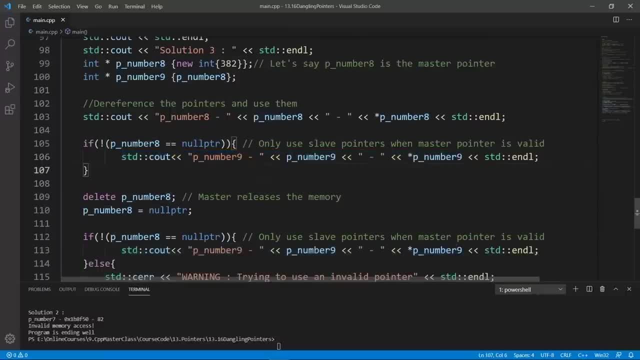 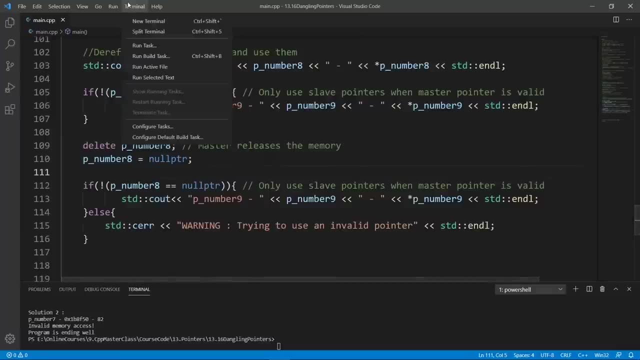 we have some valid data inside. if it is no pointer, we're not going to use that and we're going to be playing on the safe side, and this is really what we are doing here. if, around this, we're going to see that the program is not going to be able to use that and we're going to be playing on the 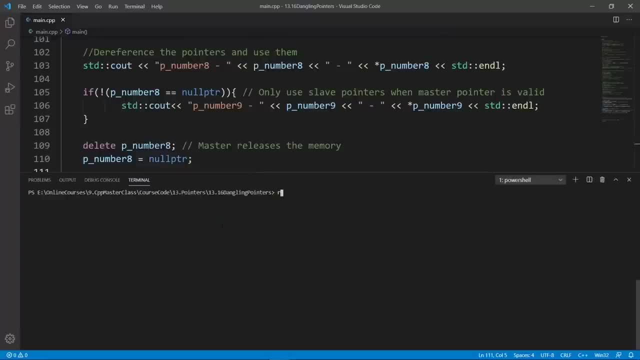 safe side and we're going to see that the program is going to end well, the world is going to be good, and if we run roaster, we're going to see that we get things printed out. we're going to go through p number eight. we're going to print stuff. we're going to go through p number nine. we're going to 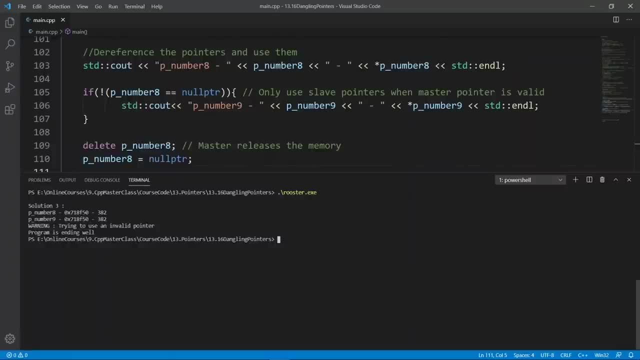 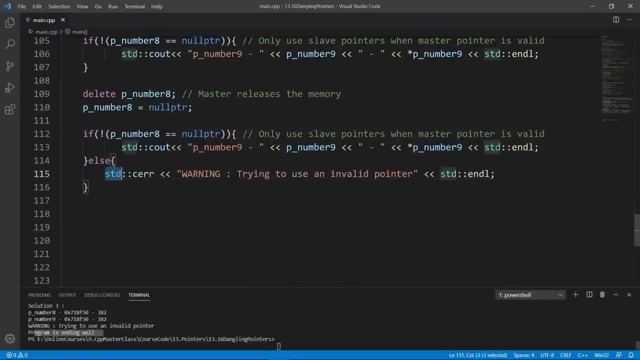 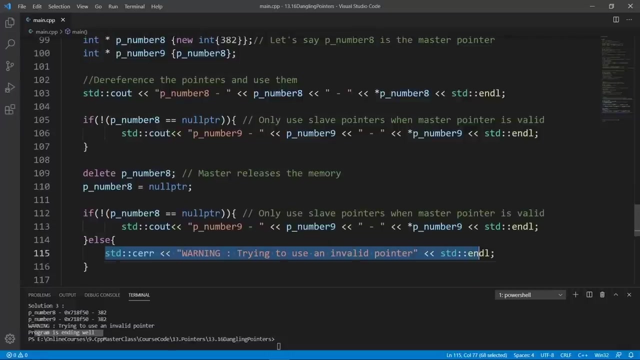 print stuff, and if we try to use the pointer after the memory has been deleted, we're going to get a clear warning that we are trying to do something really bad, and this is really what you should aim for in your c++ programs that use dynamic memory. 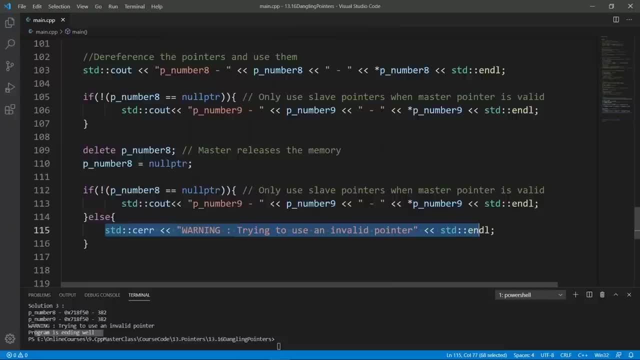 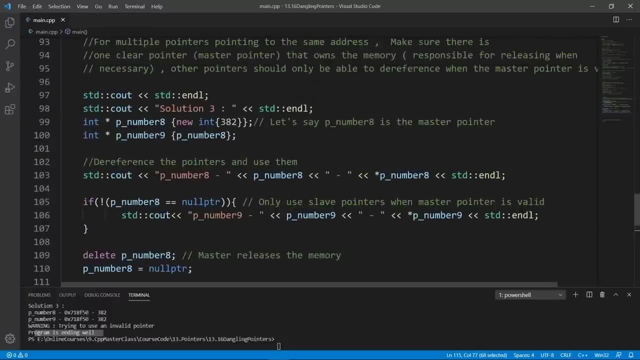 allocation and pointers. this is really all we set out to do in this lecture. i hope you know how you can avoid these problems with dangling pointers. we are going to stop here in this lecture. in this lecture, we're going to see what can happen if this new operator fails to give you the memory that you 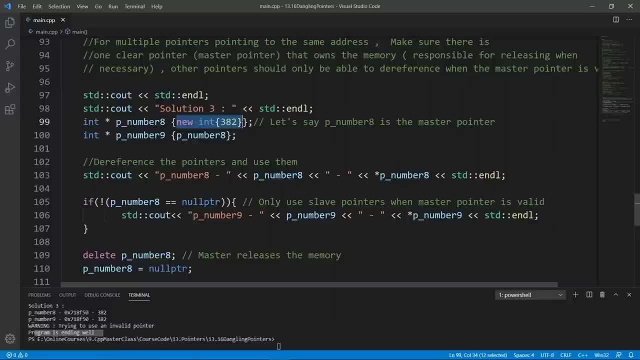 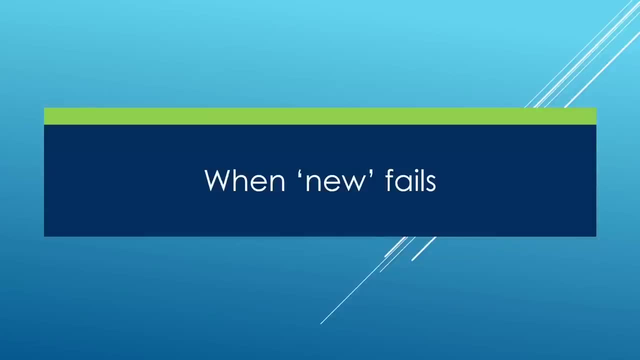 want to allocate on the heap and that's possible. go ahead and finish up here and meet me there. in this lecture we're going to explore what happens when new fails. in the last lecture we're going to see what can happen if this new operator fails to give you the memory that you want to allocate on. 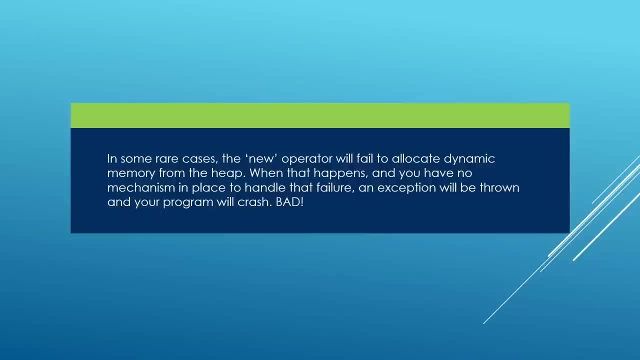 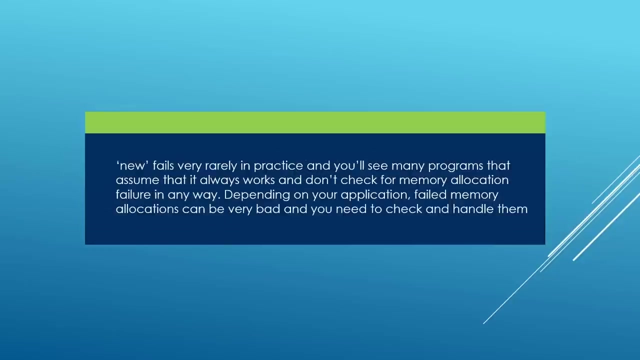 the heap and use that to do stuff, and in most cases the new operator is going to succeed. but in some rare cases it is going to fail and when you don't do anything about that failure your program is just going to crash and you might want to do something about that. i have to say that it 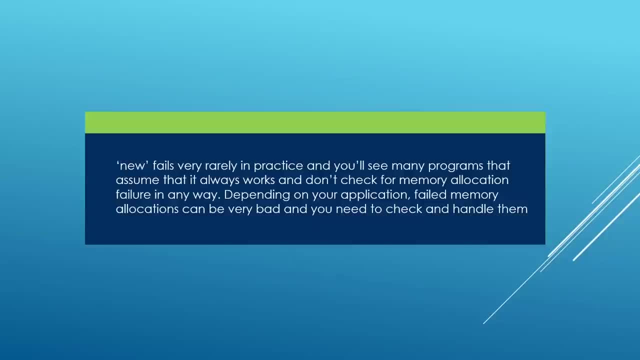 is very rare for new to fail in practice. so you're going to see a lot of code out there that's going to fail and you're going to see a lot of code that's going to crash and you're going to just uses the new operator. it doesn't really care about checking if the operation actually 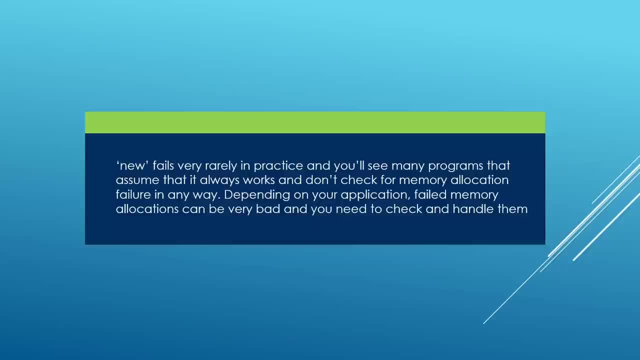 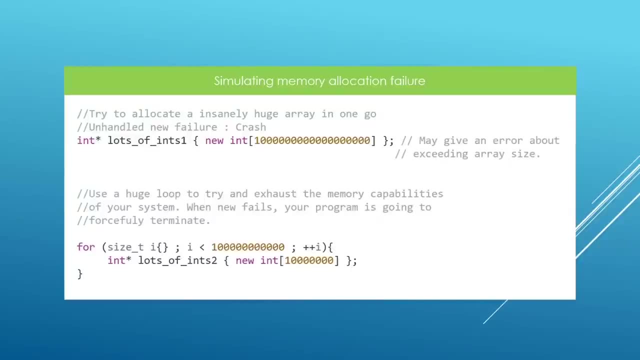 failed or succeeded. so this is a very rare case, but if you need to handle it, we're going to see how you can do that in this lecture. here is a simple example that is going to try and force the new operator to fail in the first statement. here we are using the new operator, but we are 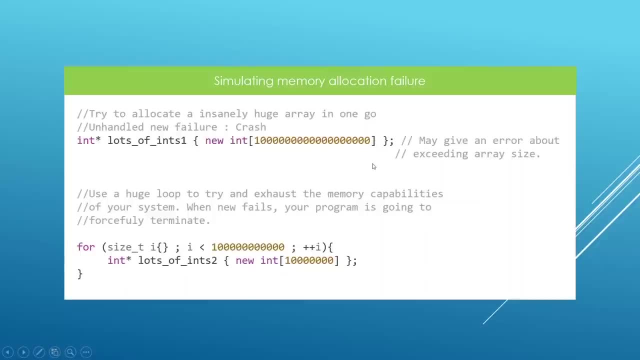 using a syntax that is going to try and allocate a lot of code that is going to fail and that is going to create a lot of integers in one go. you see that it is an array, but we haven't really seen how we can use an array like this. so just think of this code as a piece of code that is going to 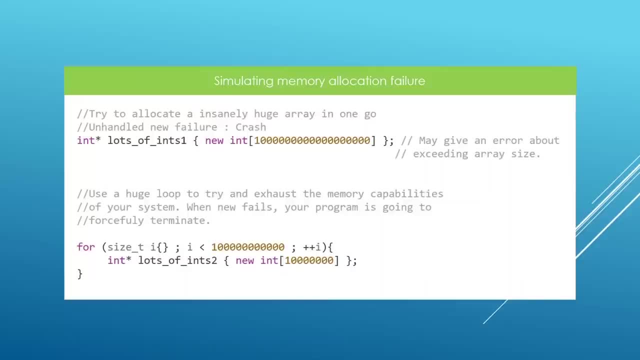 allocate a lot of integers in one go, and we're going to try and make this fail. i have to say that this may give you an error on some compilers saying that you are exceeding the array size. if that's the case, no problem, we're going to find another way to get this new operator to fail. 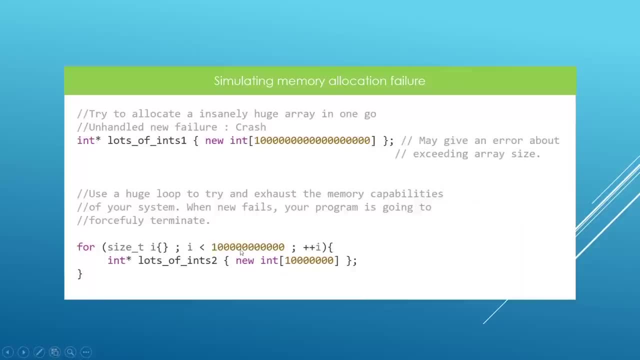 we are going to put a thing like this in the new operator and we're going to put a thing like this in a loop, and we're going to loop a lot of times enough to exhaust the heap that is allocated to our program here, and when that happens, you're going to see that the program is going to crash. 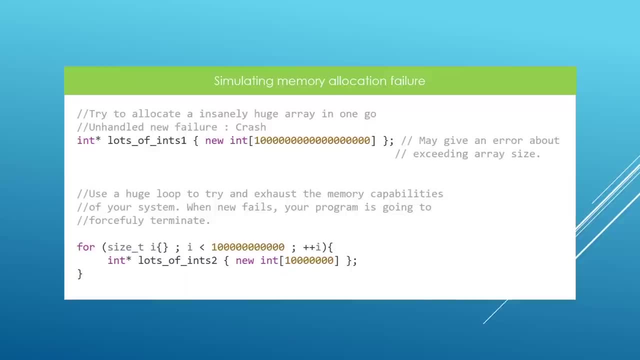 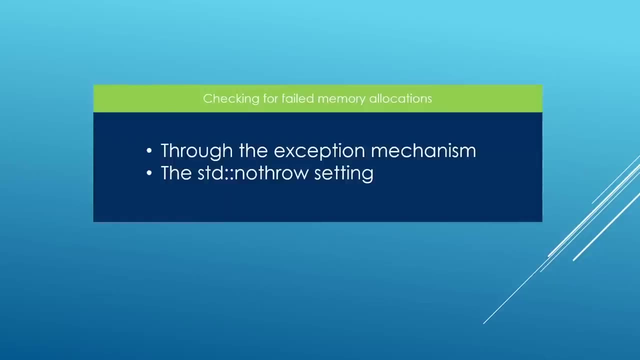 and it is bad. so new can fail and if you need to play on the sub side, you're going to handle that problem. and we have two ways we can handle this problem. we can go through the exception mechanism. this is a built-in way we have in c++ to 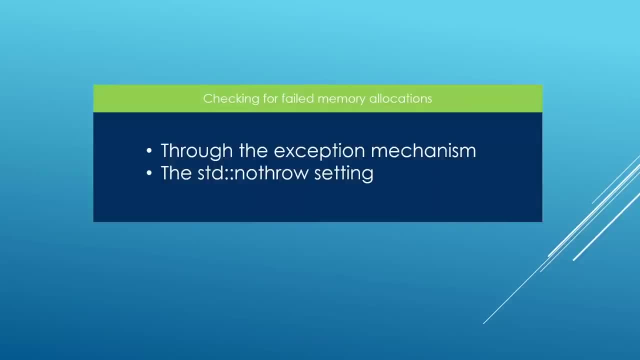 check for errors and handle them. we can also use the std no throw setting in our new operator and force it not to throw an exception, and it's going to give us no pointer if the allocation fails. i know this might sound cryptic right now, but we're going to see an example shortly and you're going to 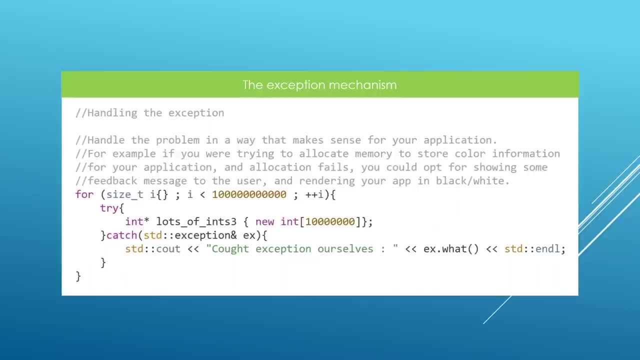 understand this. let's look at how we can use the exception mechanism. the exception mechanism is there in c++ to let you handle problems when they arise, and the way you use that, you wrap code that is potentially going to give you problems in try and catch blocks. you see here. 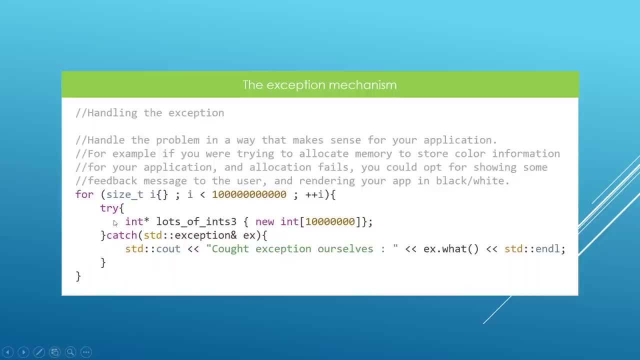 inside the loop we are saying try and inside the try blocks we have the code that could fail, we have our new operator and in the catch block you see we have a catch block. here we're going to say that we have a problem and we have a way of catching the problem. and if you look at this thing, we have 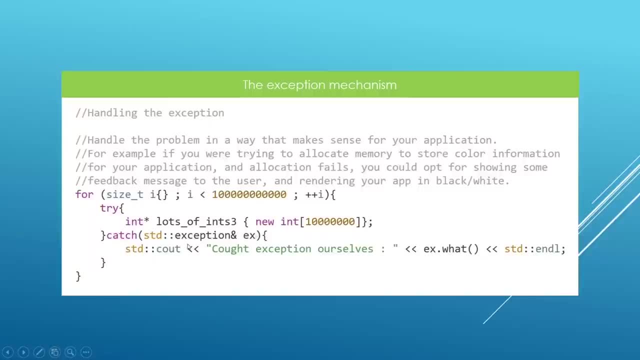 in this parenthesis: after catch we have an dow duty variable and we can ask it what kind of problem happened leading to this exception happening in our code. you can think of this like this: i realize we haven't really talked about exceptions. we are going to talk about them later in the course. 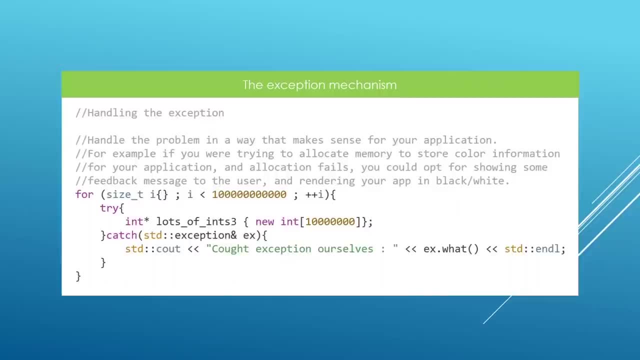 when we have enough tools to really understand what is happening. but now think of them as a tool to handle when the new operator fails. and you're not going to crash your program. so you're going. program will keep running, it will go through the end, but the new operation that you wanted to do. 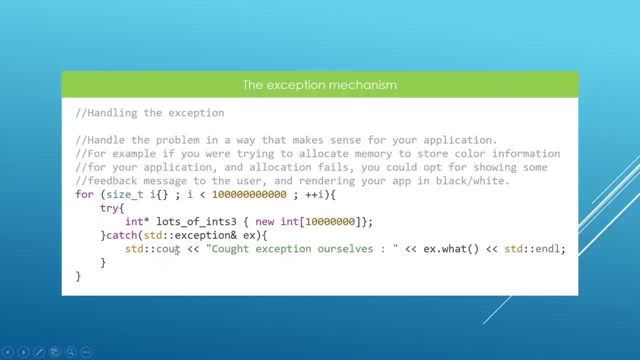 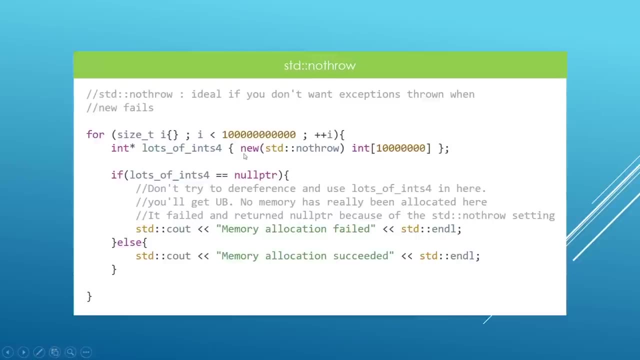 here will fail and you will be able to cache that, and this is a good thing. if you don't want to use exceptions, you can use the std no throw option, and this is a new version of the new operator you can use to tell the c++ system to not throw an exception when the operation fails. it is just. 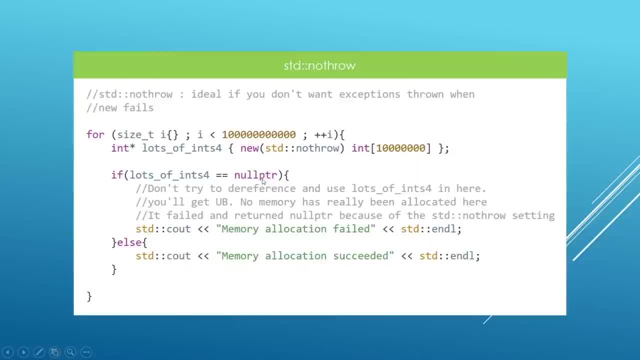 going to return null pointer and you can check for that and know that memory allocation actually failed. this is what we're going to talk about in this lecture. i hope you have an idea about this. we're going to head over to visual studio code and actually try this in action. okay, here we are. 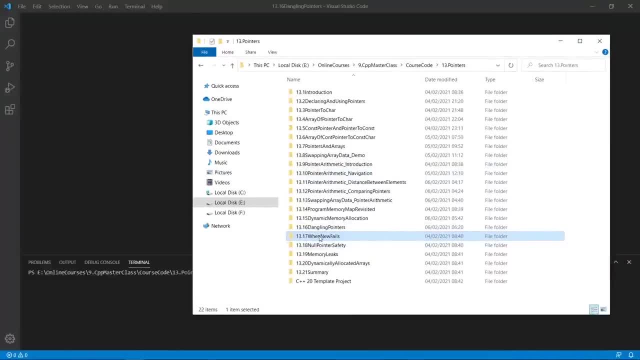 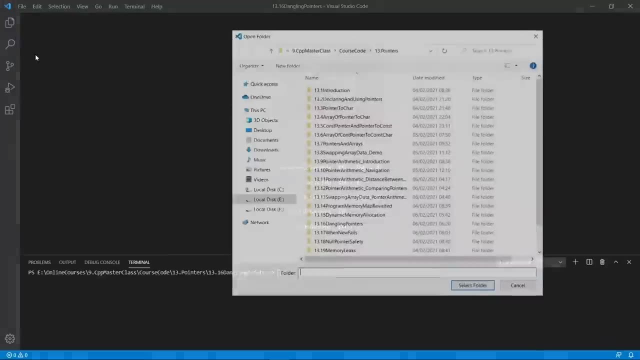 in our working directory. the current project is: when new fails, we are going to grab our template files, like we always do, and we're going to put them in place. so when new fails, that's the lecture. so we're going to do that and open this in visual studio code pretty quick and we are going to try and allocate a large 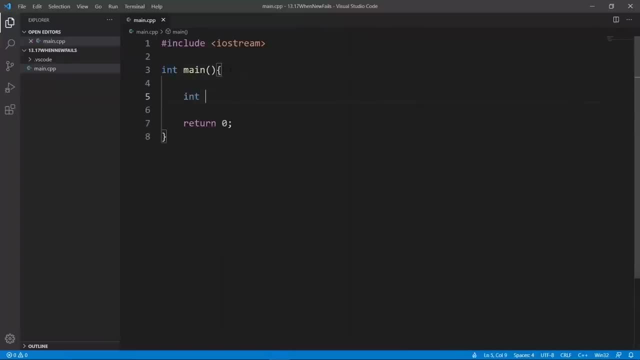 piece of memory in one go. so the way you do that, we can do, say end pointer, let's call this data, it really doesn't matter. and we're going to say new and and we're going to say that we want a huge amount of events, let's try and do that. and we're going to go down and say program ending well to. 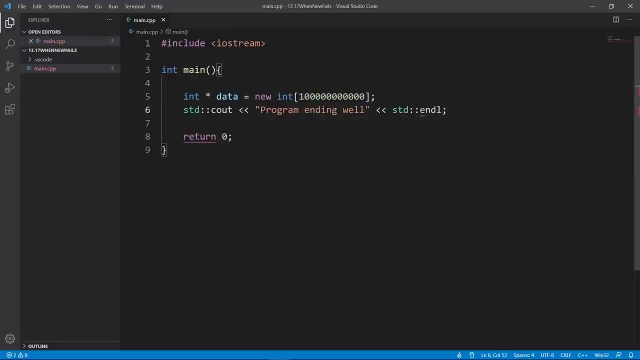 make sure we know when we are ending this program properly. so let's try and compile this. we're going to bring up a terminal and we are going to world with gcc, as we always do, and the build is going to be good. let's try and increase this. 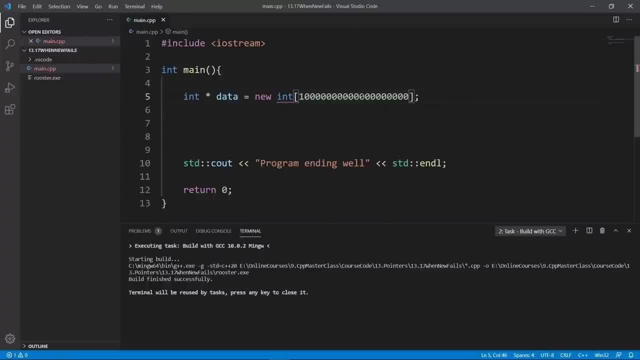 number and push it to a really big number, and you see that we have made visual studio code mad here. array is too large so they can't really allow us to do a really large array in here. okay, so let's bring this down a little bit, and if we're trying to compile this, we're going to bring up a terminal. 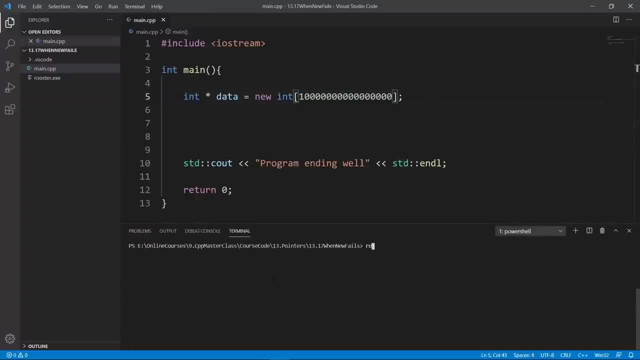 and we're trying to compile. the build is going to be good and if we run rooster, you see that the program is going to not end well. okay, so this is really a case where new fails. we can't really allocate this much on the heap storage that is allocated to this program here. remember when we 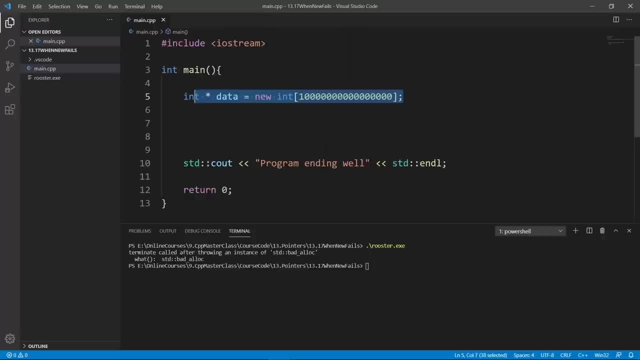 revisited the memory map idea, we saw that each program is going to have its own memory map. the memory map is going to have a lot of sections inside. we have the stack, we have the heap. our heap is not infinite so we can run out- and we just ran out with this allocation that 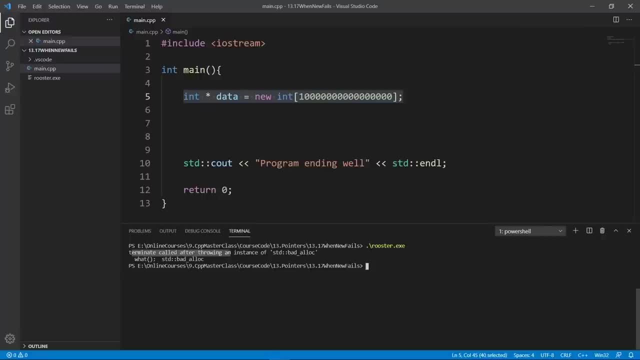 we did here and our program is going to terminate immediately. you see that it is not ending well, if this is not working, for whatever compiler you are using, we can go and do this through a loop. so what we can do, we can comment this out and we can really loop many, many times enough to exhaust the 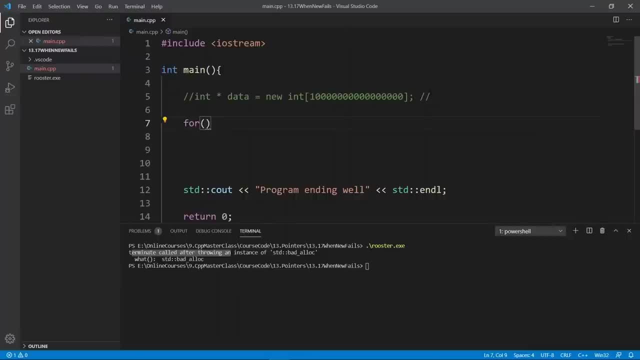 memory that is allocated for this process here, roosterexe in the memory map in the heap section. that's what i mean. and if we do this at some point the program is going to fail and we're going to get the same problem here. so let's build again. we're going to 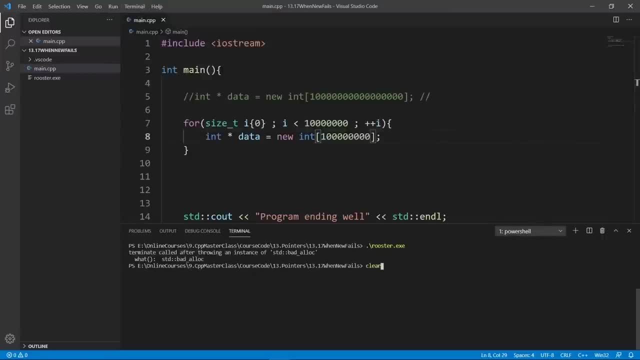 build with gcc and we are going to clear and run rooster and we're going to see it's going to loop, loop, loop and it's going to fail. we're going to see the failure in a minute and we need to find a way to solve this problem. we have seen that we have two options. let's comment on that and we're. 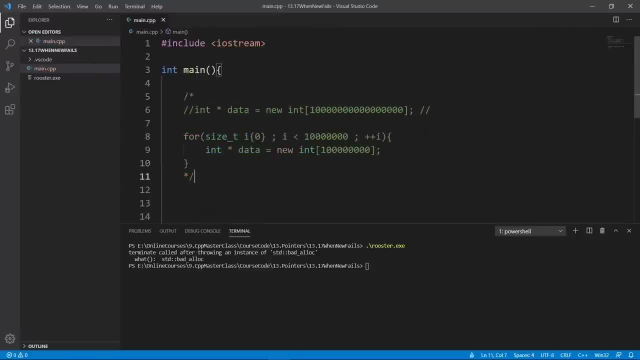 going to comment this out and look at those solutions here. the first option is to go through the exception mechanism. we can also use the std no throw option. we're going to try the exception mechanism first and what we do is wrap possibly offending code in, try and catch blocks and we're. 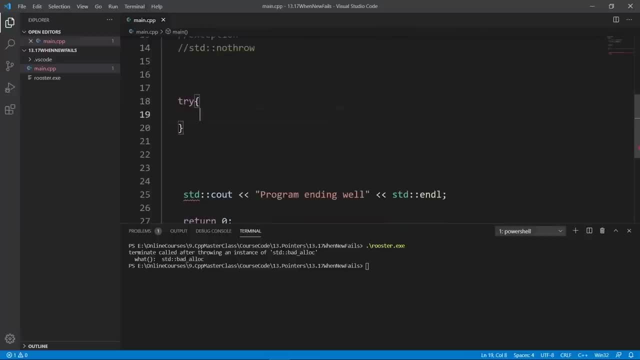 going to say try here and put a block, and we're going to say catch and we're going to say std- exception, and we're going to put an ampersand symbol here. just use this like this and we're going to get a chance to really explain. 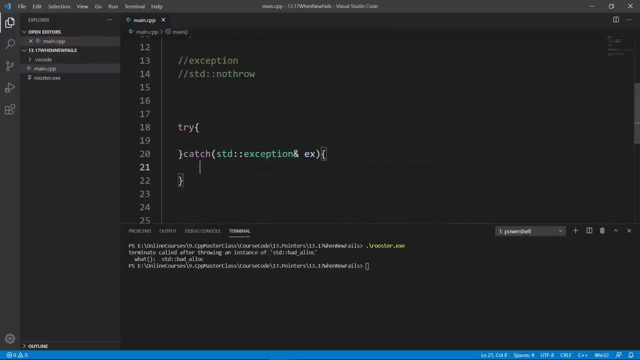 these things when we have enough tools to understand this. for now, think of this as if i have code that is potentially going to fail, like the new operator here, i am going to put that in the try block and if something goes wrong, we're going to get the error in the catch block. this is 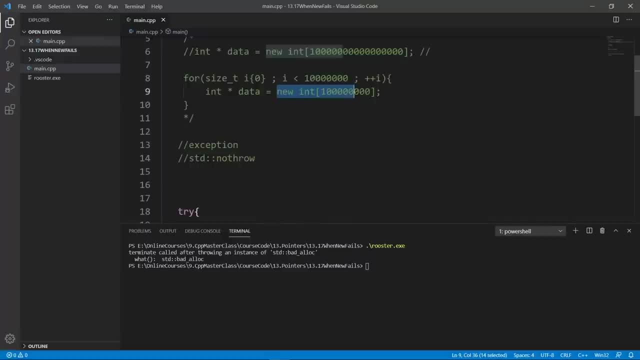 the way we do these things here. so, for example, i can take my loop here and copy it and put that down below here. okay, and i know that this line of code could fail, okay, so i am going to wrap that inside. try and catch blocks? so i am going to grab that. 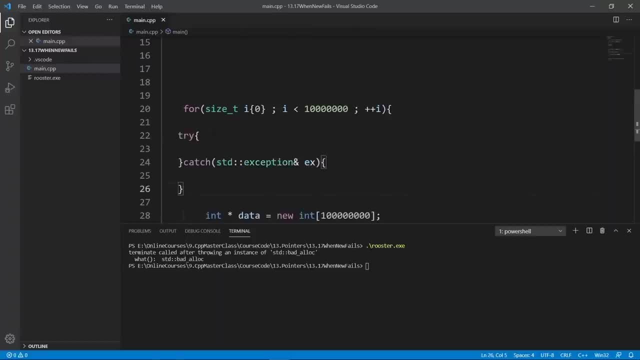 and put that in my loop. let's do that and align this a little bit and we are going to take the potentially offensive code and put that in the try block, and when the operator here fails, something goes wrong and we're going to catch the problem in the catch block. this is what we mean here again, we don't have enough tools to. 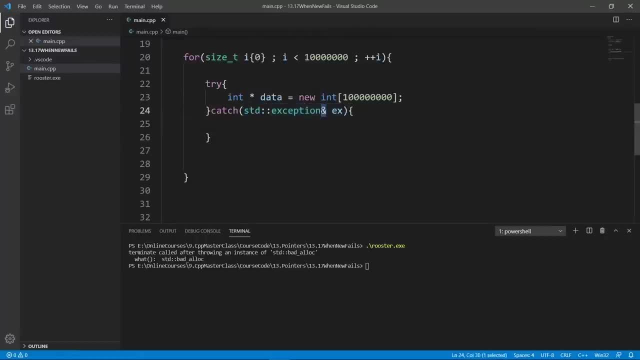 understand why we are doing this thing here. what is the meaning of this ampersand symbol? we're going to learn about that later in the course, but for now, we want to put together something good enough for this program not to crash like it was doing right here. okay, we're going to catch the error and 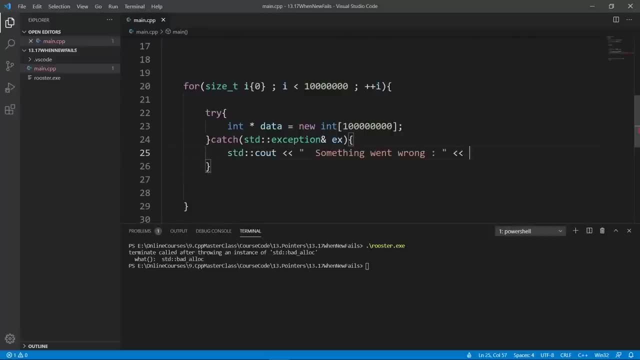 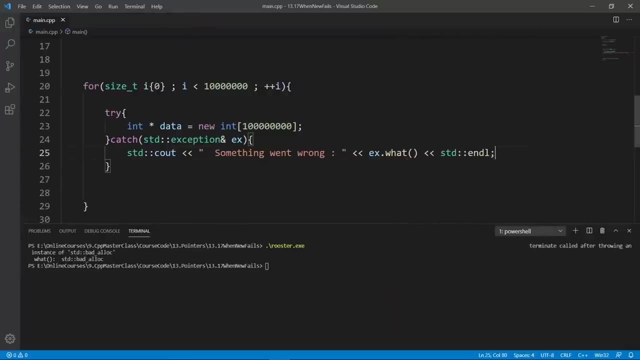 say something went wrong and we're going to print out what actually went wrong. we're going to say ex and we can call a function called what on this and we can say std endl. let's hide this pane here, because we want to see clearly what is happening here. this is how you can prevent your program from 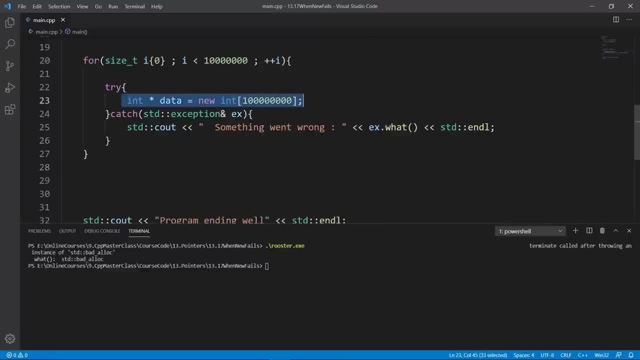 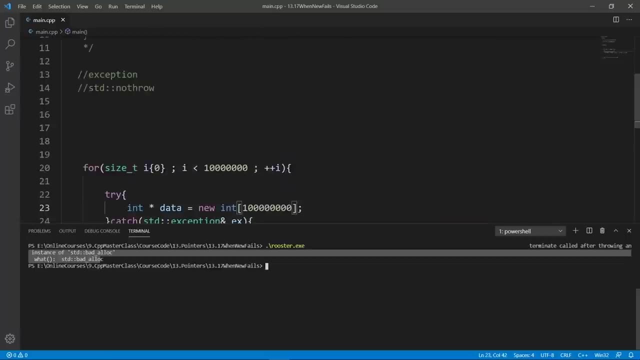 crashing and it is going to end well, because now we have handled the problem and we haven't caused a crash like we were doing down here. now we're going to try and build this code- let's bring it up a little bit so that it is not messy here- and we're going to build with gcc. the build is: 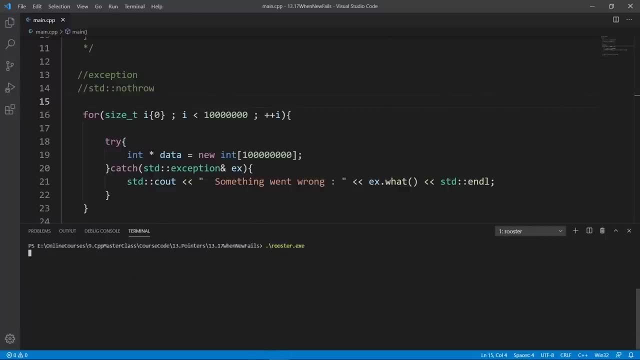 going to be good and we're going to clear and run rooster and it is going to do its thing. it's going to keep looping around and it's going to say: something went bad. it's going to hit a point where all these allocations are going to fail and if we really wait for it, it is going to end. 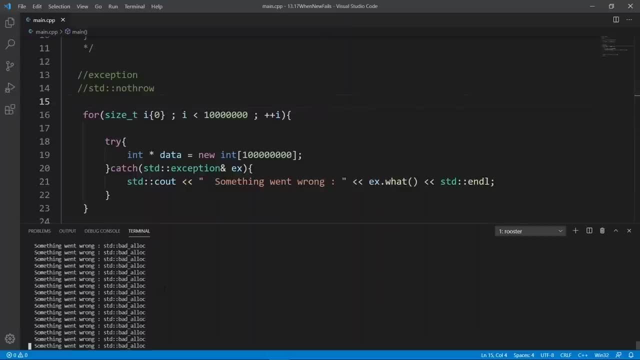 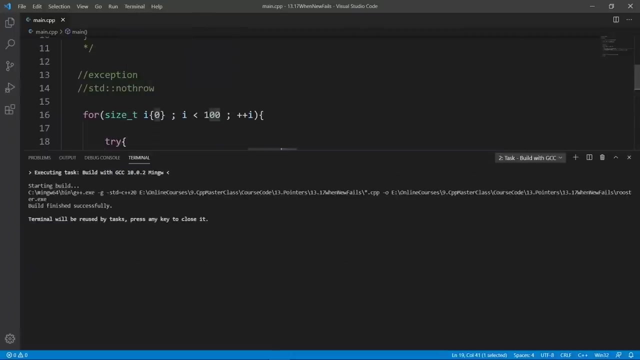 and we're going to see that it's going to end. well, let's try and hit ctrl c and terminate it, because we don't want to wait for this amount of time, and let's bring that down to 100 and increase this number here. let's see if that actually works. so we're going to build. for now we just want to see that the 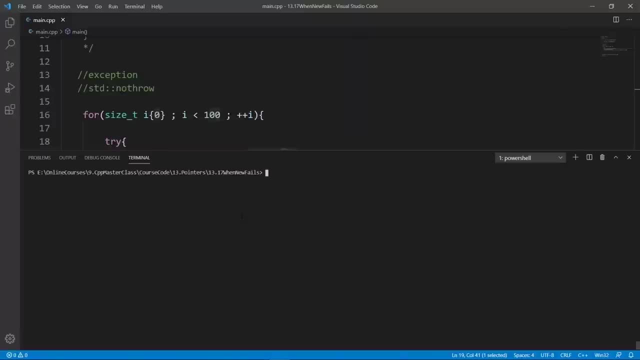 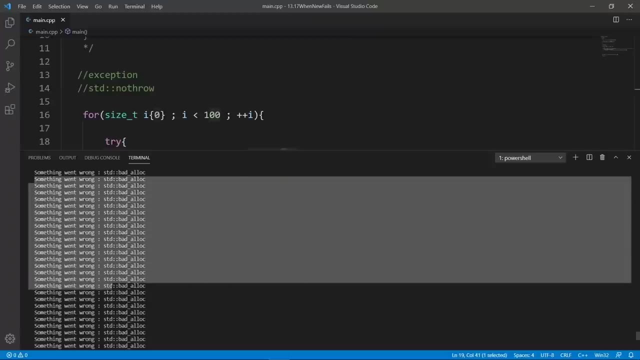 program is not really crashing. so we're going to run rooster and you see that it's going to keep running and at some point it's going to fail to allocate memory and it's going to say something. and it's going to fail to allocate memory and it's going to say something, and it's going to say something. 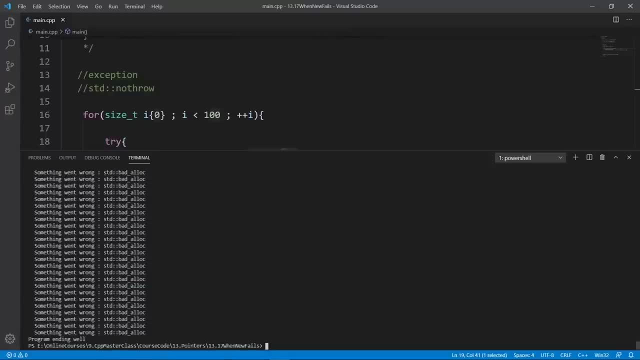 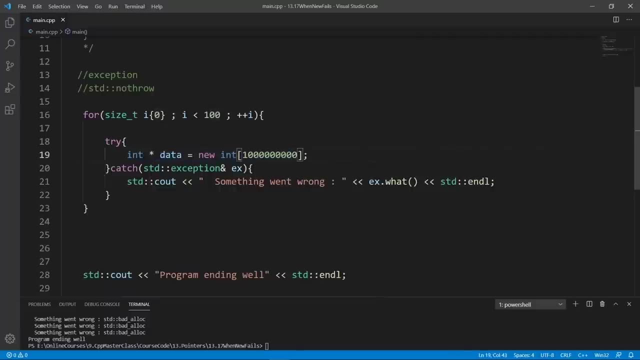 went wrong, but if you keep going down, you're going to see that the program is ending well. so what is happening here is that the new operator actually failed, but we code the problem and could handle it in here. so what is called handling the problem? you're going to handle it in whatever makes. 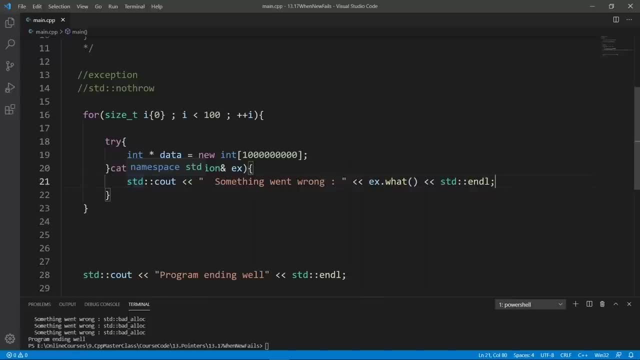 sense in your program. if we were, for example, trying to set up a color in some uh widget in your application and the color fails, and you fail to set up the color, you may show your user interface in black and white and keep running your program instead of getting across. this is just a. 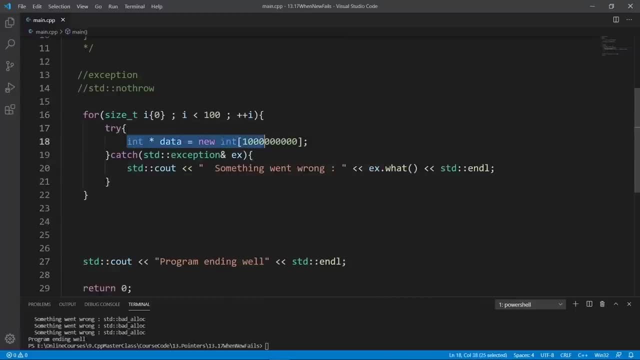 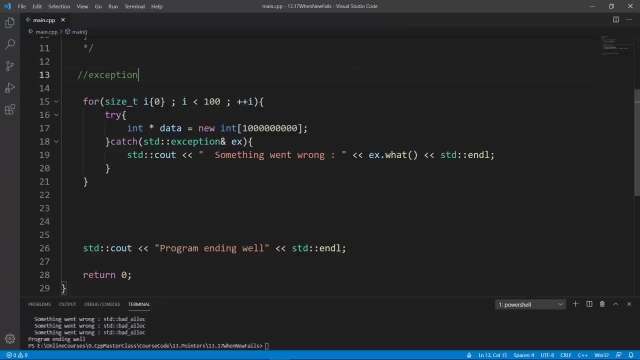 way to show you that you can handle stuff when new fails. this is one way we can solve the problem, so we're going to look at the second way. the exception mechanism is the first, so we're going to comment this out because we're going to see another way, and let's do that. we can also use the. 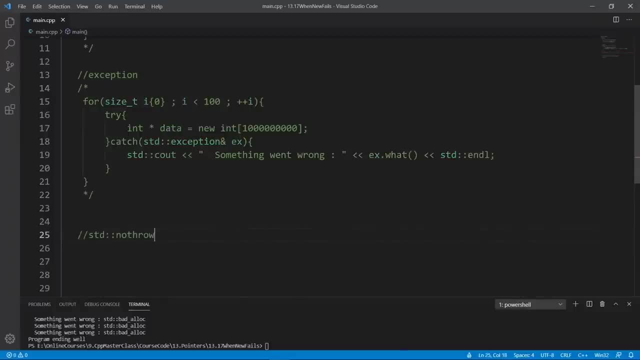 std: no throw setting on our new operator when we are allocating for new memory. so we're going to do that and we're going to bring up our loop here. we're going to reuse that for this. here we're not going to be using the exception mechanism, so we're going to do 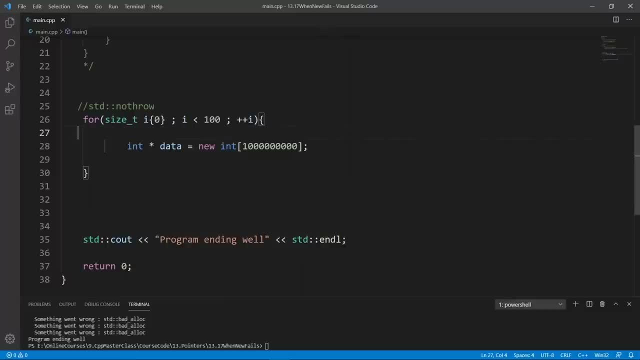 something like this: get rid of the try and catch block. but we're going to still be in our loop here. so what we can do is pass the new operator a parameter and say std, no throw. and when we do this, if new fails we are going to get null pointer stored in data here. so we 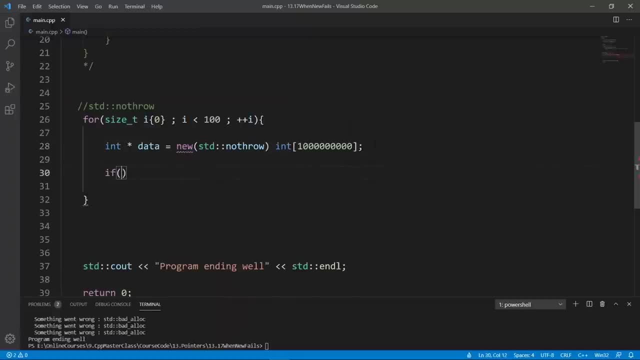 can check this against null pointer. we can say if data is different from null pointer and we can do whatever we want to do. we can do that and say: stdc out data allocated and we can try and compile this program. so what we're going to do is run this through our compiler, through gcc. 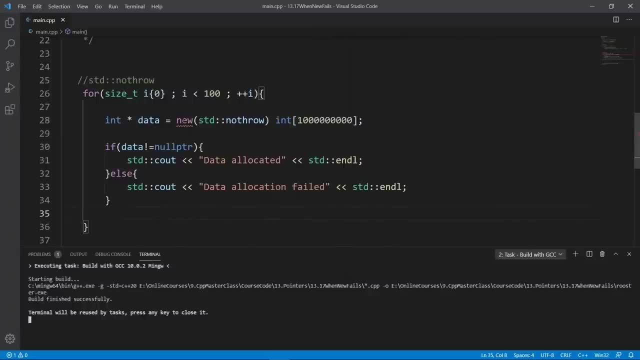 and you're going to see that the world is going to be good. and you see that visual studio code was giving us a squiggly line because it can't really understand this, but this is going to go through the compiler and it is going to work exactly how we expect. so let's try and run this. 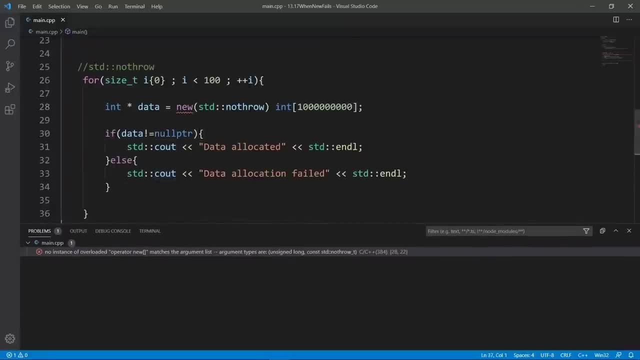 program. we're going to ignore visual studio code for now, because the world was good, we could build with gcc and we saw that this was welding successfully. so we can clear- let's clear- program in the simulator and we're going to send it out to this worldcom, something like that. so we'll 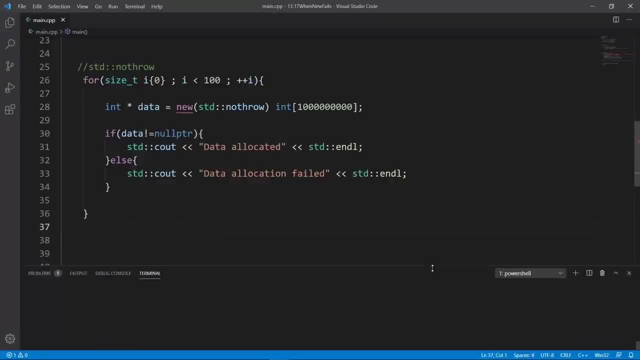 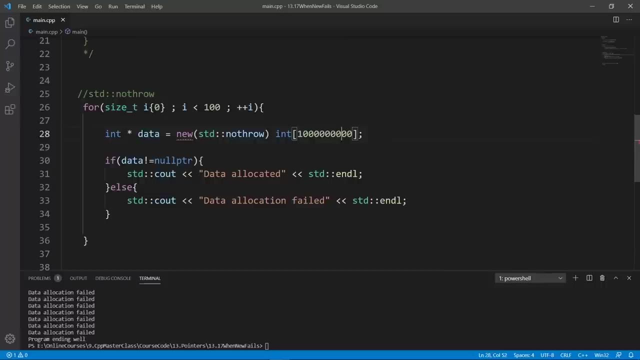 save this as our new operator and you can see that the program is not crashing because we can go through this program and it's going to run the program properly and run rooster and it's going to say data allocated a few other times and the program is going to end. you see that the program 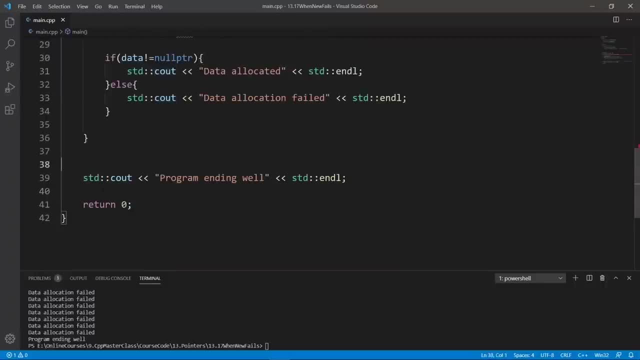 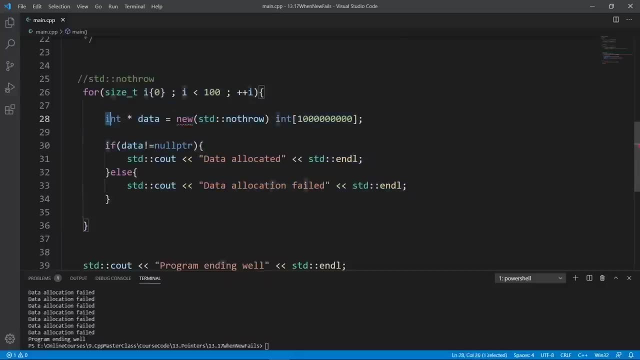 is not crashing because we are also handling the problem, but we are going through a new mechanism to do that and that's using the std no throw option with our new operator here things. when new fails, you can either go through the exception mechanism by using try and catch. 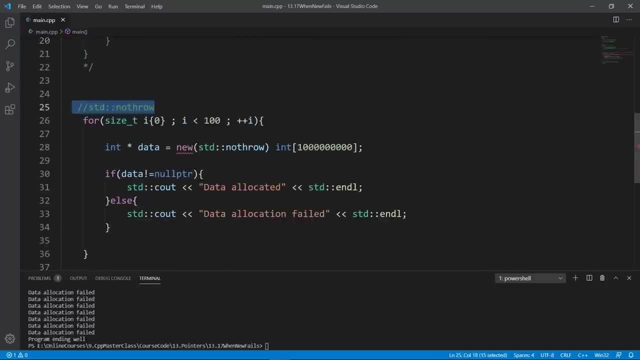 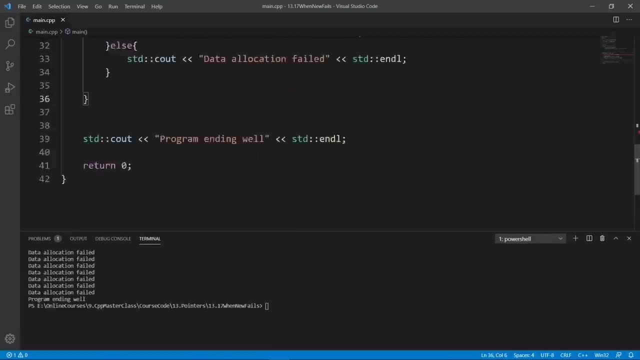 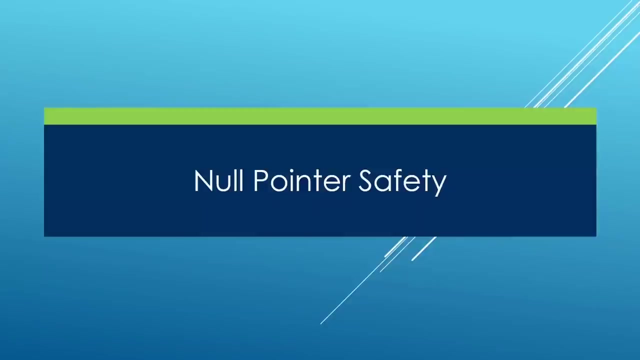 blocks, like we did here, or you can use the std no throw option. we are going to stop here in this lecture. in the next one we're going to learn about null pointer safety. go ahead and finish up here and meet me there. in this lecture we're going to explore the concept called null pointer safety. 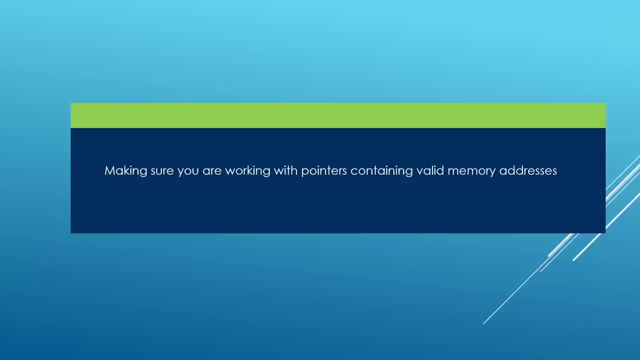 and this is a series of measures you take to make sure that when you are using a pointer, it contains a valid address. if you don't have a valid address inside, you don't use that pointer, and we do that through a series of checks we can do against null pointer, for example. here we have 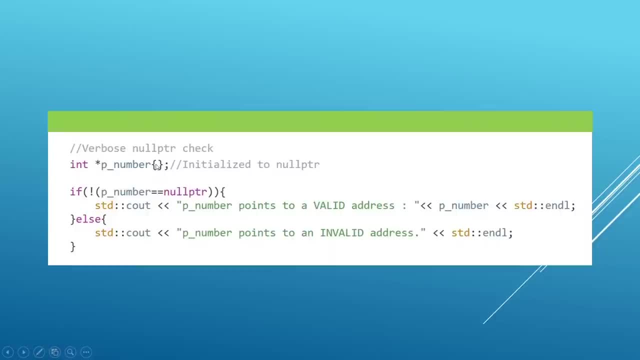 a pointer that is initialized to null pointer implicitly through braced initializers, and what we can do is check if p number doesn't contain null pointer- and this is how we say it in c++- and if it contains null pointer, we're not going to use it. 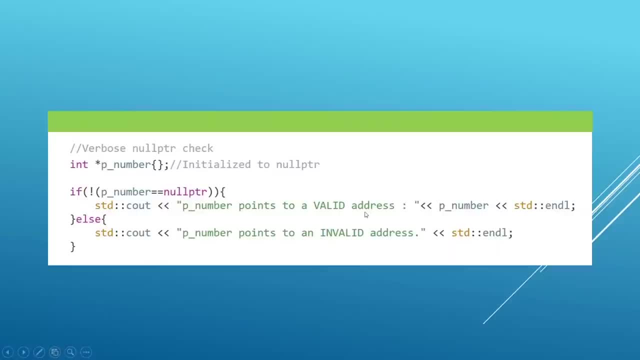 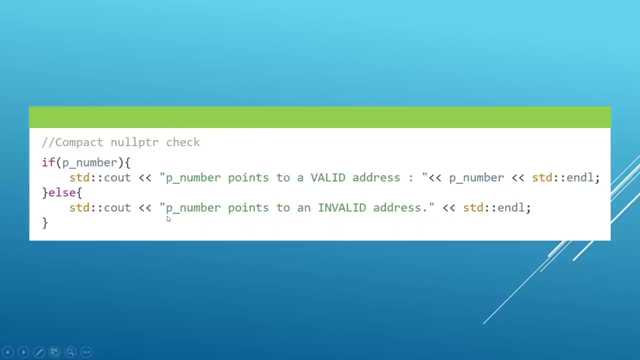 we're going to say it points to an invalid address. this is something you can do. it is simple in nature, but it is going to save you lots of trouble. this is one version we can do this and but we can also directly plug in p number and use it like this: if it contains null pointer, we're going to get. 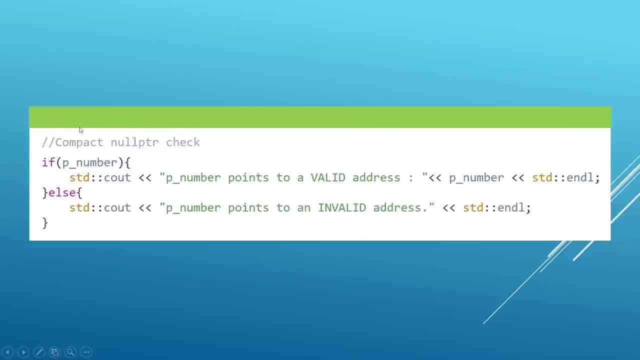 the message printed out that we have an invalid address. if we have something other than null pointer, we're going to have a valid address, and if it contains null pointer, we're going to get valid address and we can do something with that. this is going to work, because a pointer can also. 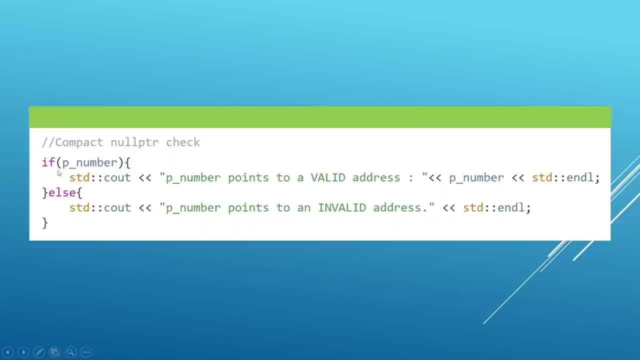 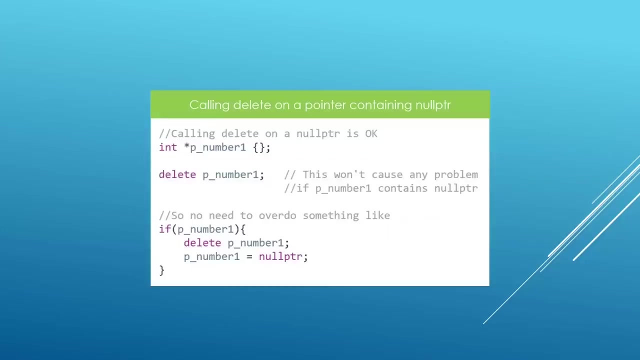 be implicitly converted into a boolean expression that our if statement expects here, and it is going to work exactly how we want here. so we're going to see this in a minute when we hit visual studio code. before we do that, though, i want you to be aware that you can call delete on a pointer. 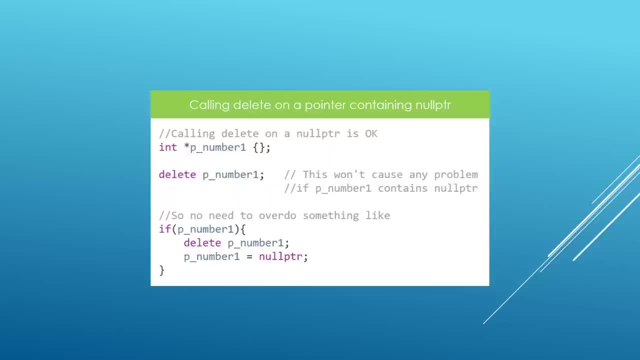 containing null pointer without doing the check. here it is going to be okay. we have seen many rules about pointers and many students will develop an intuition that you have to check for no pointer before you do anything on your pointer. and they even do that before they call delete. i have to. 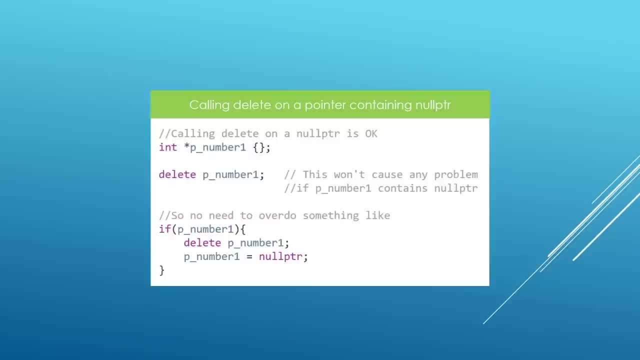 break it to you that it is safe to call delete on a pointer that contains no pointer. so you don't need to do something like we have here, say, and check if p number one and then delete p number one and reset that to no pointer. this is really overkill. you can call delete on a pointer and 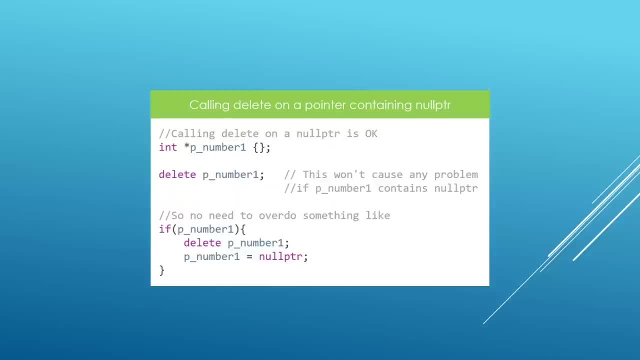 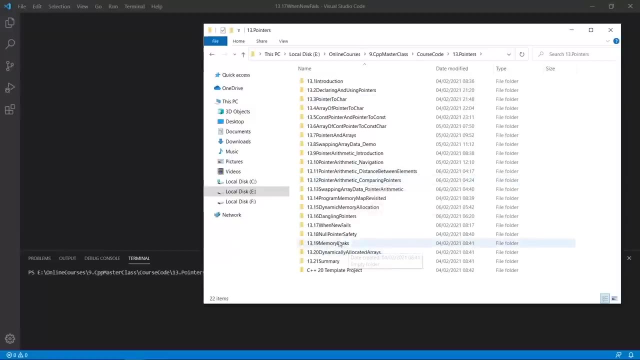 it is going to be fine, even if it contains no pointer. now we're going to go to visual studio code and see these things in action. here we are in our working directory. the current project is no pointer safety. we're going to grab our template project and we're going to put that in the current project that we are interested in and we are going. 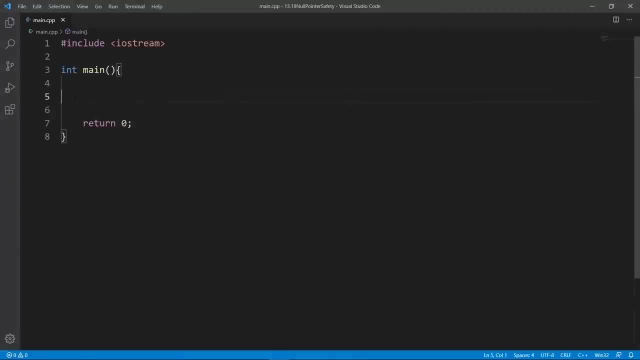 to open this in visual studio code open folder and we are going to put in a verbose no pointer. check what we are doing here is nothing new. we have a pointer called p number. it is a pointer to end and it is initialized to null pointer through implicit initialization, here using 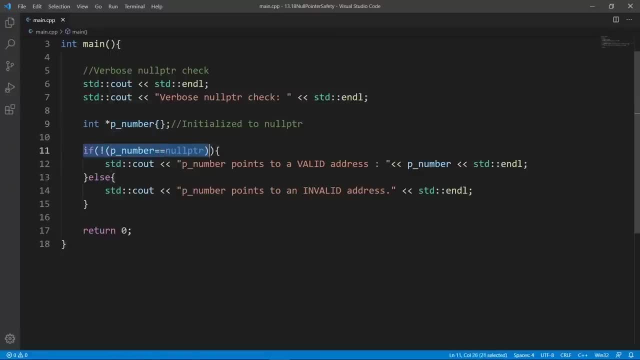 braced initialization and we are checking to see if it contains no pointer. if it does, we're going to say it contains an invalid address. if it doesn't, we're going to say that it has a valid address. and you see that we are using a negation here. you can do this however you want, if we're. 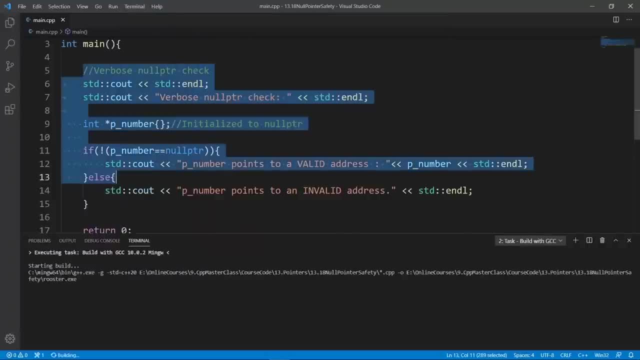 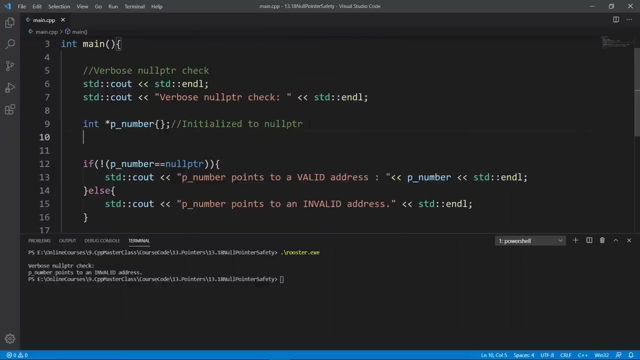 trying to build this with gcc. let's see what we get. the book is going to go through the menu and if we run rooster we're going to see that p number points to an invalid address because it contains no pointer. but if we try and set up a new variable, for example, and say p number, 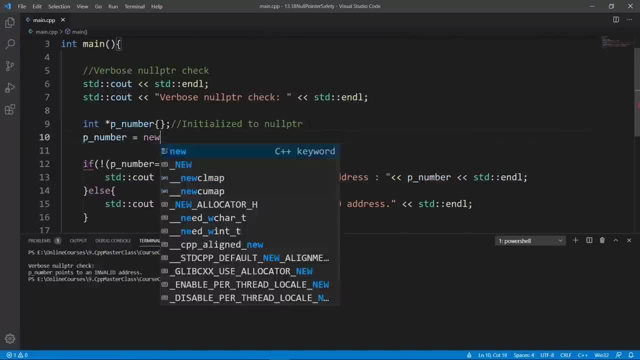 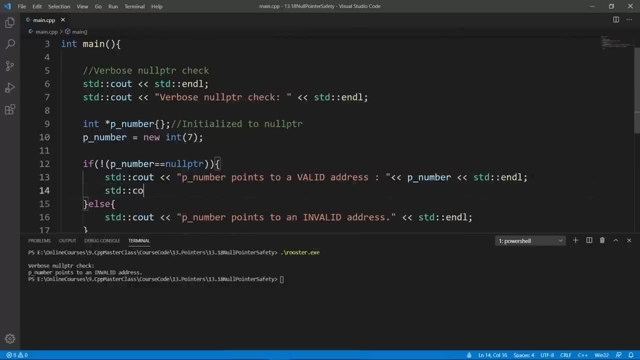 and let's use dynamic memory- we have learned about that- and initialize that with a seven, for example, and when it points to a valid address, we're going to print whatever is in there. we know how to do that, so we can say p number and we're going to print whatever is in there. 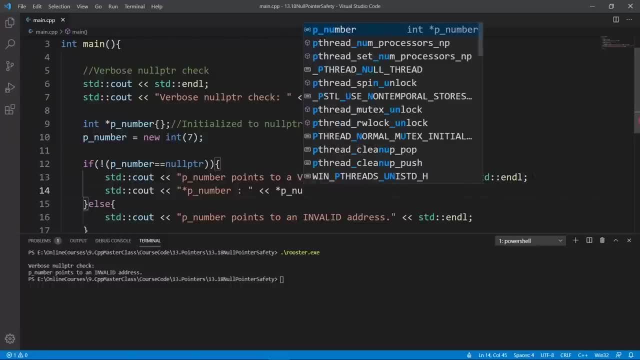 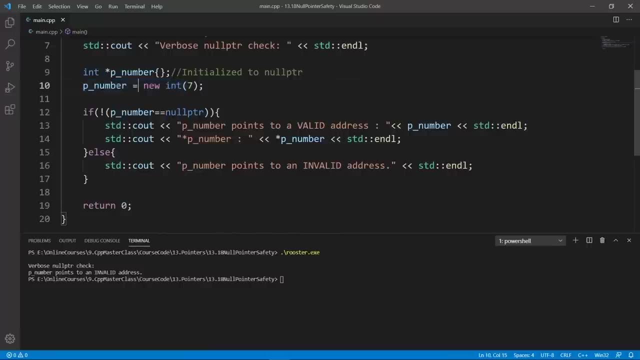 to print whatever is inside and say p number through the referencing, and we're going to say std and dl. now the pointer is not going to contain no pointer because it contains the address of the memory that was allocated on the heap here. but once we do that we have to remember to release. 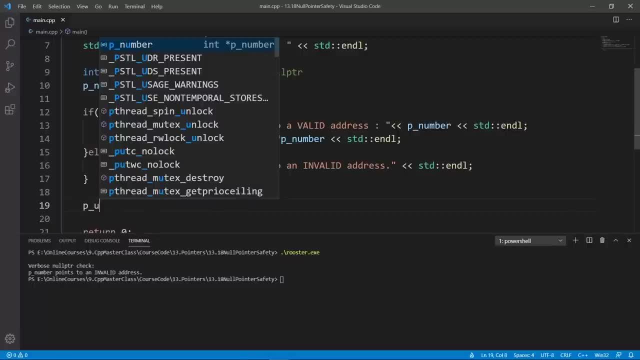 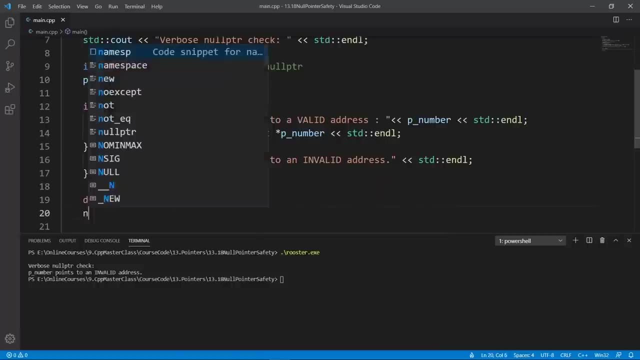 this memory. so please remember to release your memory after you are done using it. so we're going to say delete p number after that and we need to reset it. so we're going to say delete p number to no pointer. in this case it really is useless because nobody is going to be using this pointer. 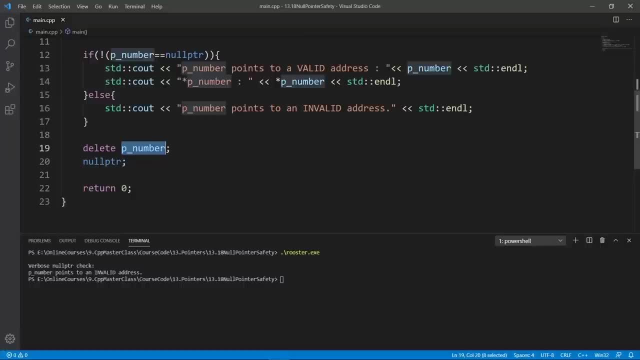 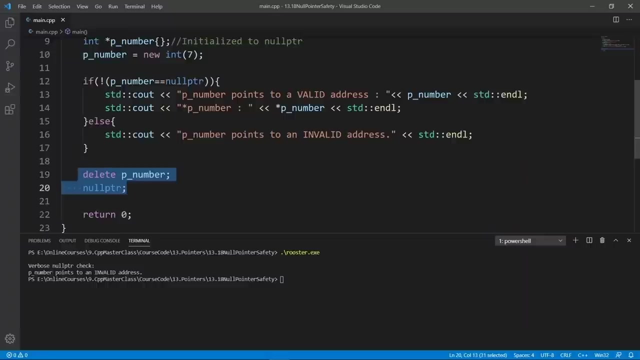 anymore. the program is about to end, but it is a good practice to do this even in this case, because once this way of doing events is burnt into your memory, it has become your habit. you're going to be writing cipher c++ code now. we're going to try and run this, so we're going to build again. 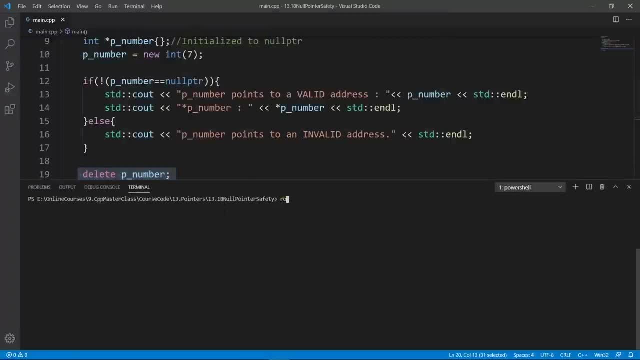 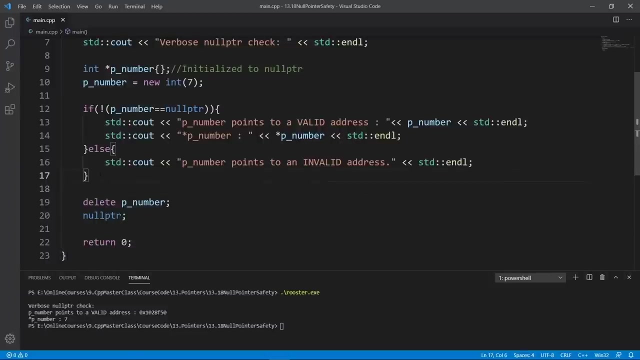 the build is going to go through and it is going to say that we have valid address in memory. which is this guy and what is inside is a 7, and now we are writing safer c plus plus code through null pointer safety. here we can also do a direct check using p number. 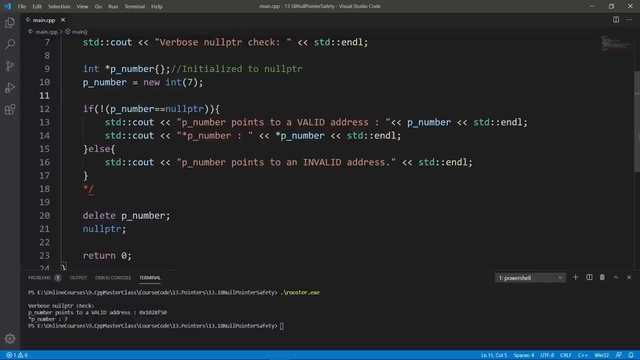 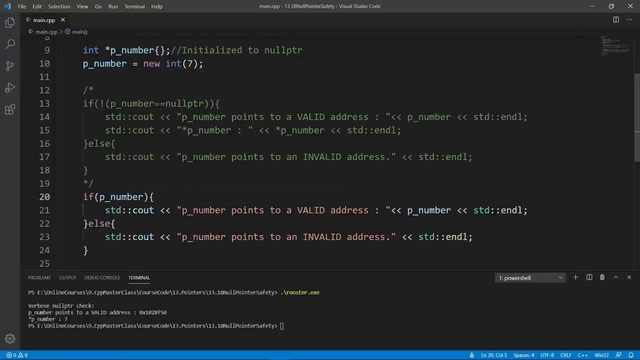 without checking if it is equal to null pointer, because this is verbose, but it is something you will see in practice. you can also do something like this and say: if p number, and you're going to get exactly the same thing. so if we have some valid address inside, we're going to print. 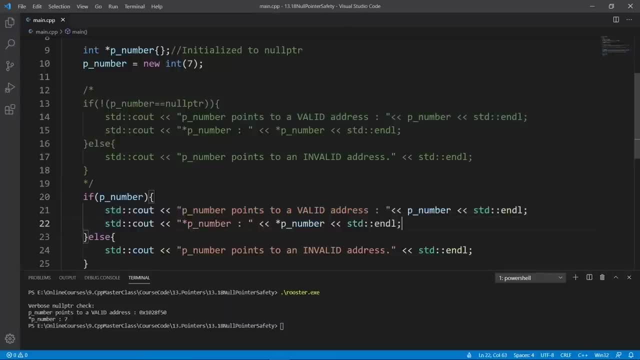 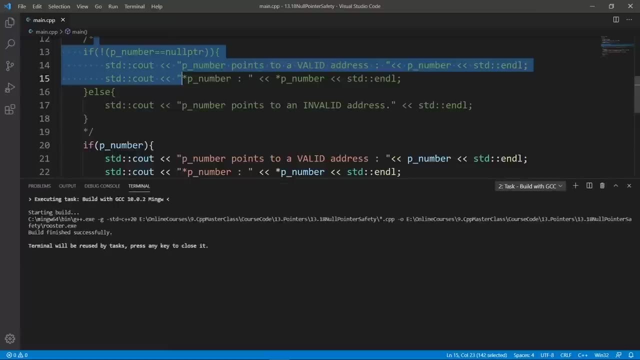 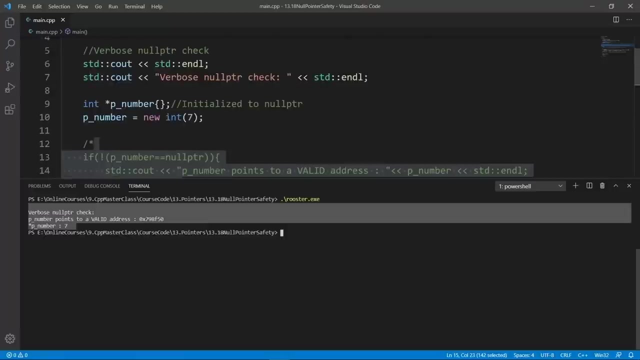 that let's print the same thing as in the previous code here and if we build and run, we're going to get exactly the same thing, okay, so let's clear, because the build is good. let's clear and run, rooster. you see that we get exactly the same thing. and if we didn't? 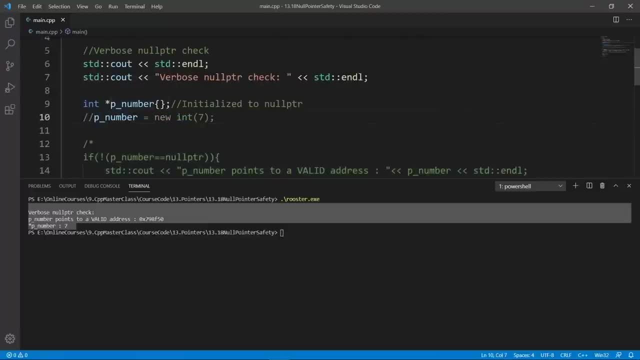 initialize this guy with the new dynamic piece of memory. we're going to get that the memory is invalid, the address we have in the pointer is going to be invalid and we're going to print that out through our code. here we run rooster- invalid address. okay. 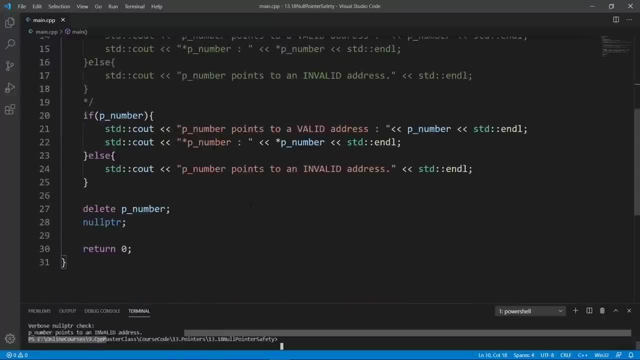 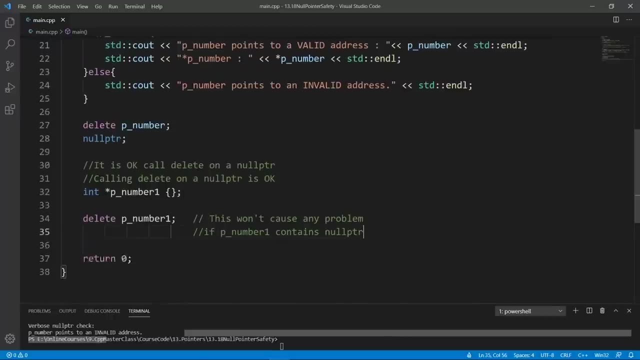 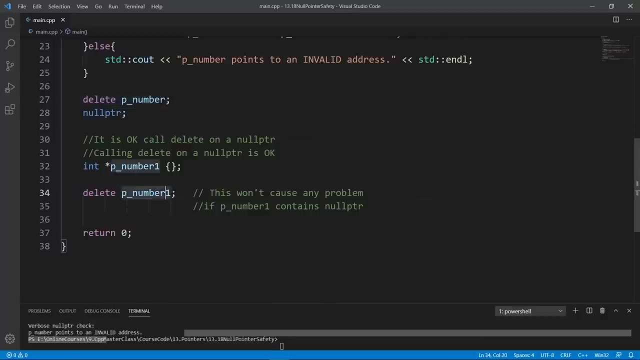 the last thing i want you to see is that it is okay to call delete on a null pointer, and we're going to say that here. so we're going to go down here and put in a piece of code. we are setting up a new pointer, p, number 1, initialized with null pointer. if we call deletion, this is going to work. 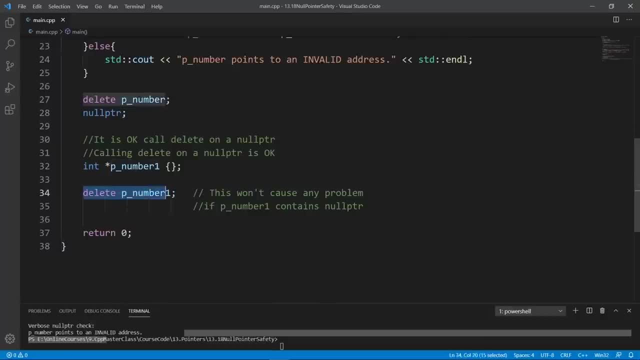 well and you're not going to get a crash or anything. this is valid C++ code. so if we try and compile this, it is going to work fine and you don't really have to do a null pointer check before you delete like this, because that's overkill. 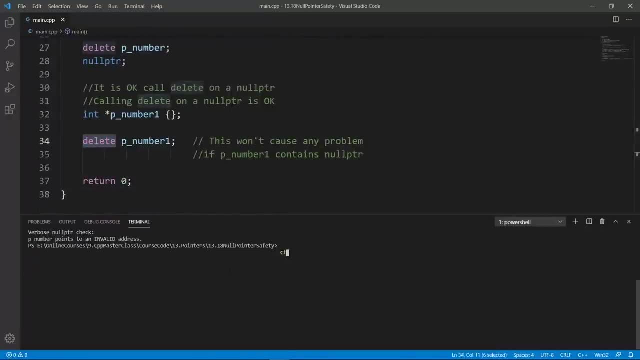 you see that the program works successfully and we can clear and run it and we're going to get exactly the same things we had before. so some people are going to do something like they're going to check for null pointer and they're going to say if P, number one, for example, is not equal to null pointer, and they're 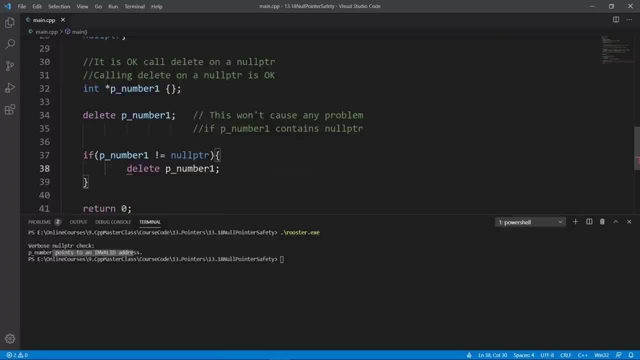 going to say something like delete here and they're going to do something like this and this is going to work. but it is really overkill. you don't need to do this test because it is safe to call delete on a pointer even if it contains no pointer in the first place, so you don't need to do things like this. this. 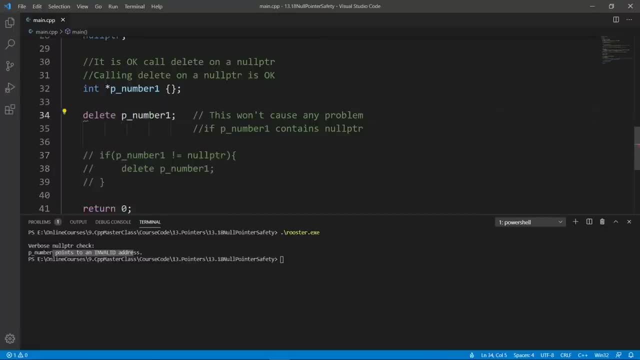 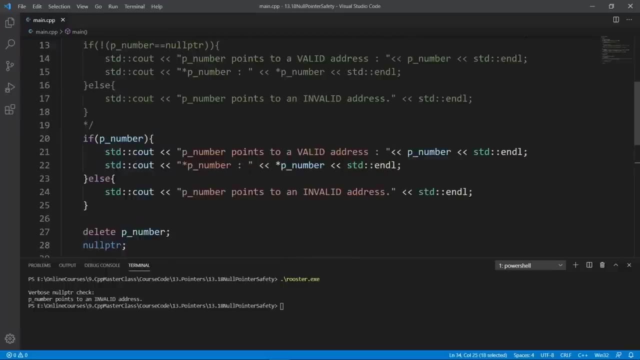 is going to work just fine. don't be afraid to call delete on a pointer because it will not work. if you delete it on a pointer, it might contain null pointer. this is really all we mean by null pointer safety and I hope I gave you a few examples to make this pretty clear. we are going to 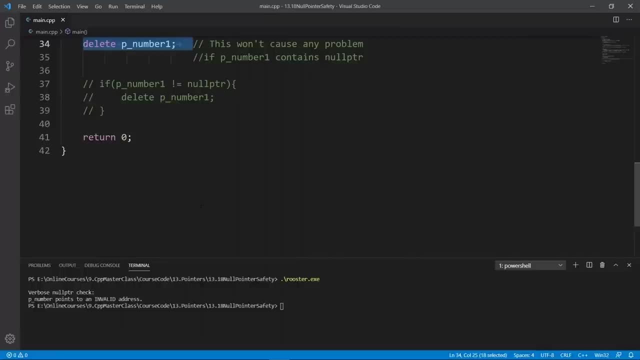 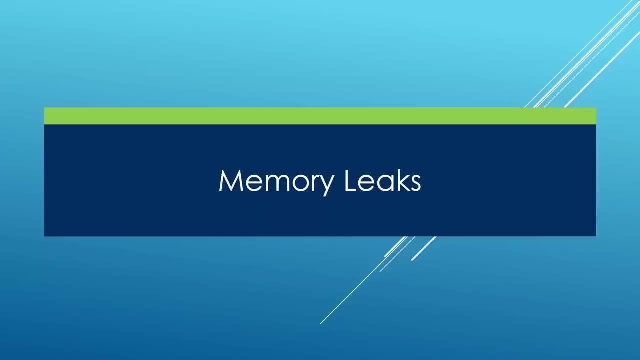 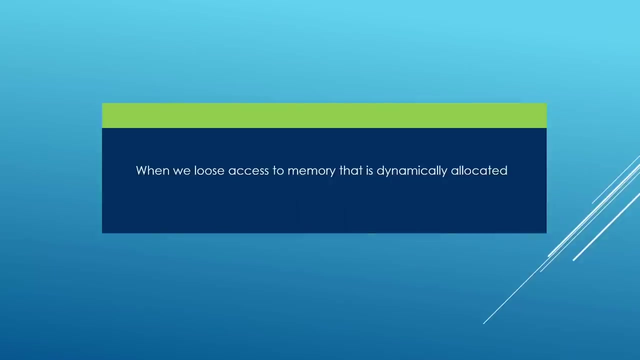 stop here in this lecture, the next one we're going to learn about memory leaks. go ahead and finish up here and meet me there. in this lecture, we're going to learn about memory leaks, and a memory leak is when you have lost access to a piece of memory that was dynamically allocated to your 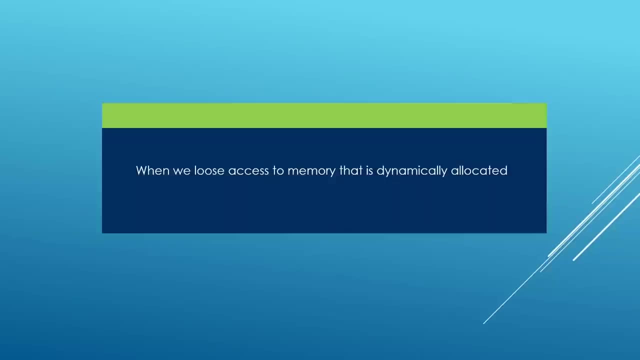 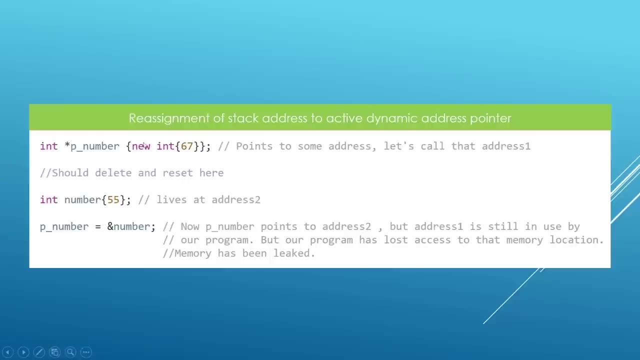 program, you basically lose the pointer that was pointing to that dynamically allocated piece of memory. here we have a few examples of that. for example, here we have P number, which contains a dynamically allocated piece of memory which is going to contain an integer. it's going to be 4 byte, the value inside. 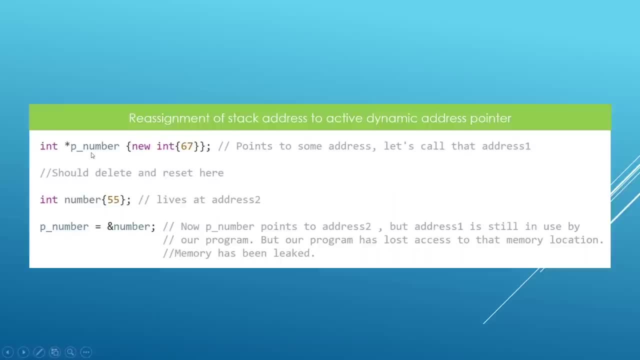 is going to be a 67. this P number is our only key to manipulate that memory and it is the key through which we even go to release that memory and return that to the operating system. but notice what we do down here. we are setting up a new. 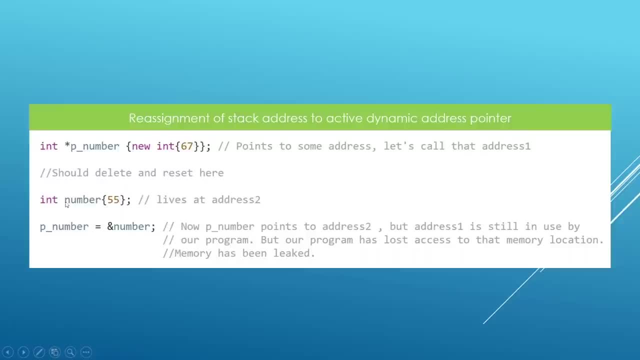 number variable. it is an integer and it is allocated on the stack because this is a local variable. it's not a pointer, it's not dynamically allocated and we take the address of number and assign that to our pointer. the moment we do that, we have no way to release the memory that was allocated to P number in. 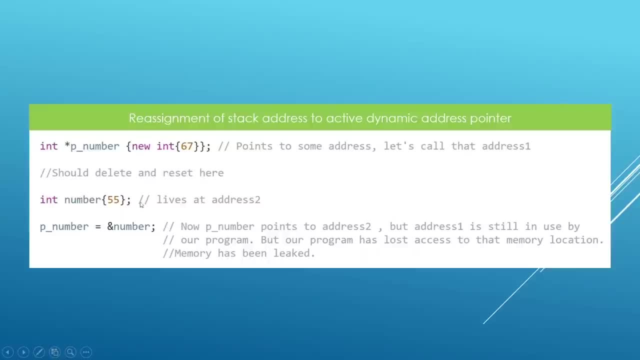 the first place, and if we do that, the operating system is going to think that this memory is ours. but we don't have a way to release this memory anymore because the pointer that was helping us access this memory has been repurposed to point to this number variable here. I hope you see that. 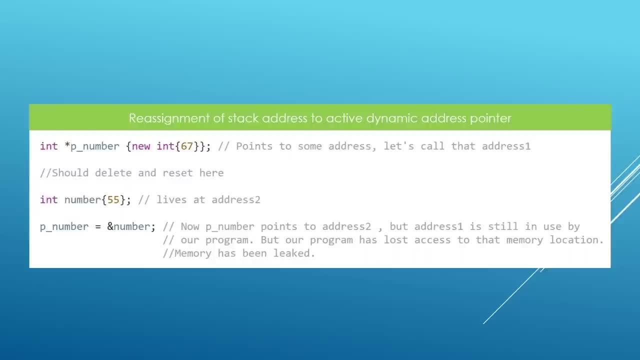 and a memory leak is something like this: when you lose the pointer that would otherwise be used to release the memory and your program is basically going to keep using this memory and the operating system is not going to have a way to send this memory, so it is useless. so you are no longer using this memory because 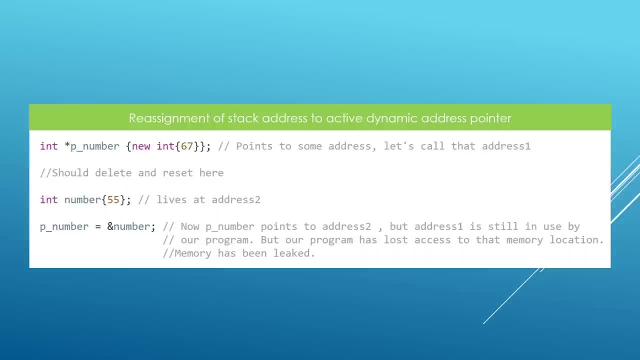 you can't access it and do things with it, and the operating system can't use it either, because it thanks. it's your memory. hopefully you can see that this is a really bad situation and you should avoid these things in your application. so do avoid memory leaks like a plague. this is one situation in which we can have a memory leak. 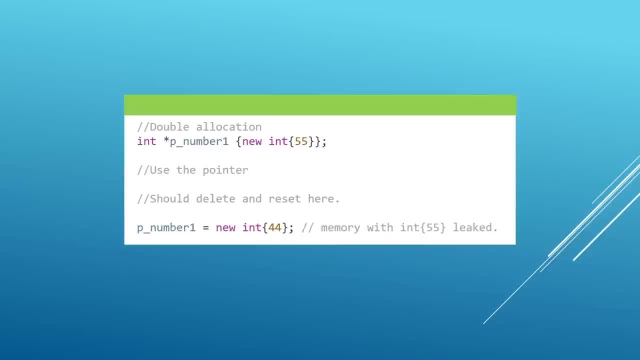 here is another example where we have double allocation. we have a pointer P, number one. it is pointing to dynamically allocated memory again and the value inside is a 55. if we use this pointer to allocate new memory, the first memory that we were pointing to is going to. 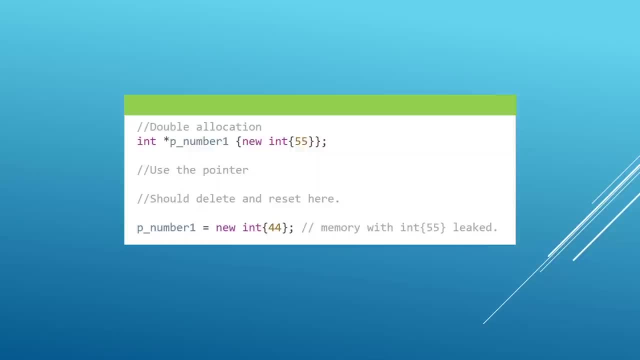 be leaked again. it is the same thing. we have lost access to the first memory. now we are pointing to the second dynamic memory that was allocated to contain the 44 here and again, this is a memory leak. your program has lost access to the memory containing 55 here and the operating system also thinks that you are using this. 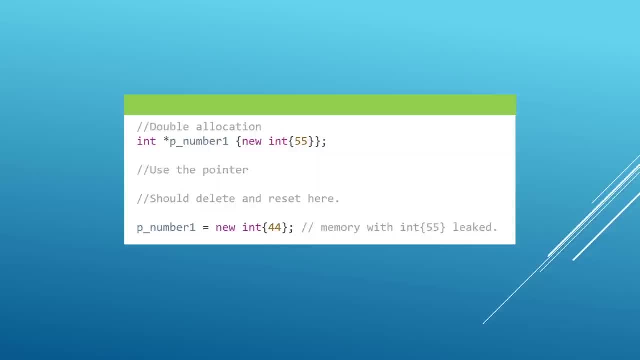 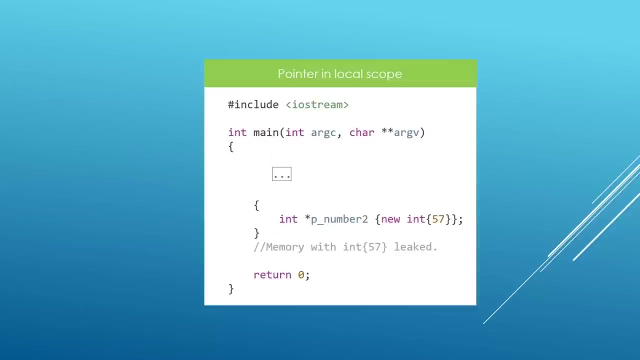 memory because you didn't explicitly return it to the operating system through the delete operator. again, memory leaks are bad. do avoid them in your programs. here is another simple example of a case where you might have a memory leak. you go in a nested scope like this and allocate a new piece. 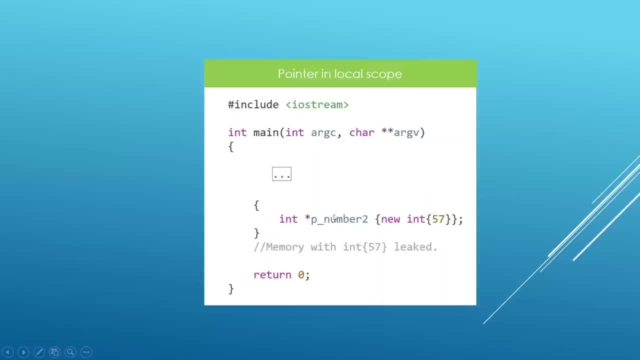 of memory- dynamically of course, and point to the memory that you are using and you can see that the memory leaks are bad. do avoid them in your programs. here is another simple example of a case where you that through P number two here. but P number two itself is a pointer and it is a local variable. 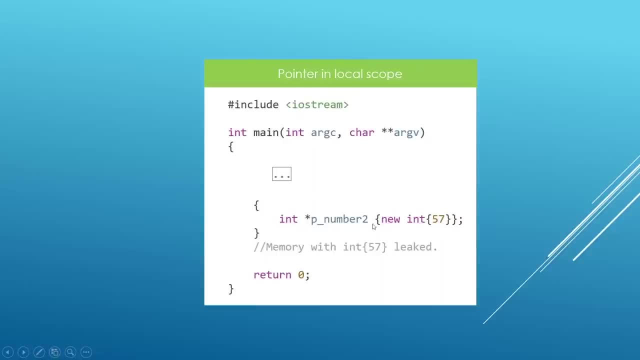 nested in this scope. when this scope ends, P number two is going to die, but the dynamic memory itself is not going to die. you just lost access to it and you can't access it again. this is a memory leak and you should avoid this in your programs. memory leaks are really bad and in extreme cases they 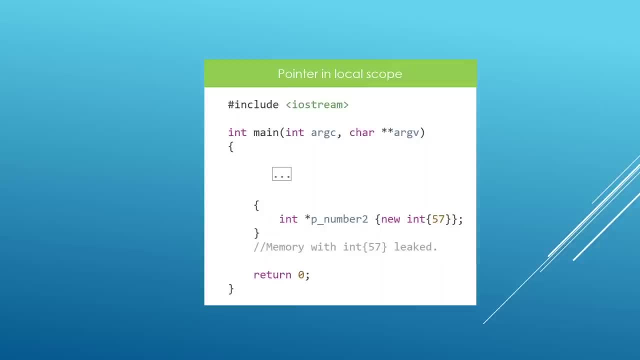 might even lead to your program crashing. if your program keeps running for an extended period of time- think of programs like those running in servers, for example. they can even run for three months without stopping- and if your program is increasingly leaking memory, the operating system is going to think that you. 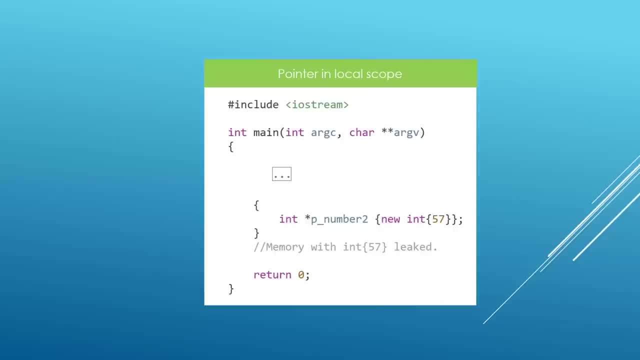 are taking too much heap memory, it's going to terminate your program, like we saw in the lecture where we learned on conditions where the new operator failed. so if you allocate too much memory, then your program can really take the next operations you're going to do with new. 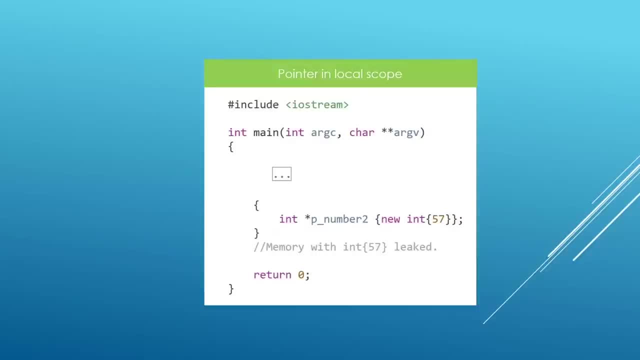 are going to fail and your program is going to terminate. the message here is: memory leaks are bad. you should avoid them in your programs and whenever you think that you're no longer using a piece of memory, make sure you delete it and return it to the operating system you're going. 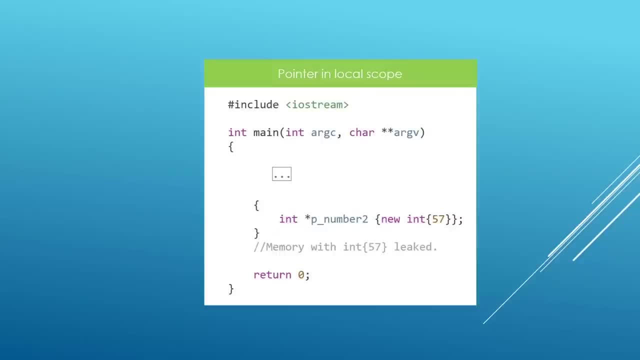 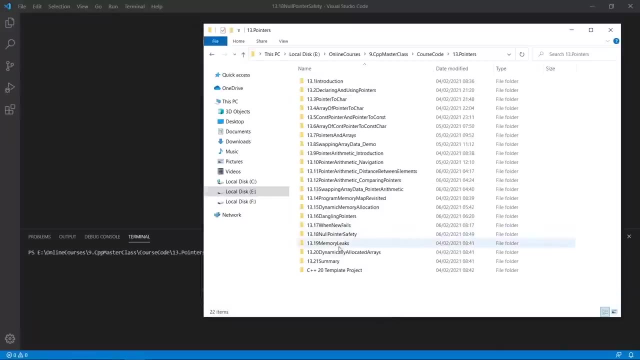 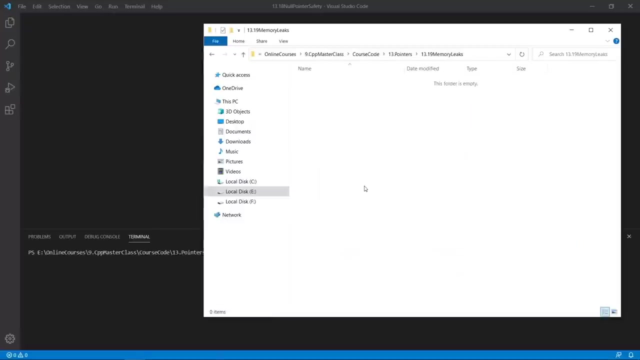 to be writing much safer C++ code. we're going to head over to Visual Studio code and actually try this. here we are in our working directory. the current project is memory leaks. we're going to bring in our template files and we're going to put them in place in the lecture on memory leaks and we are going to open. 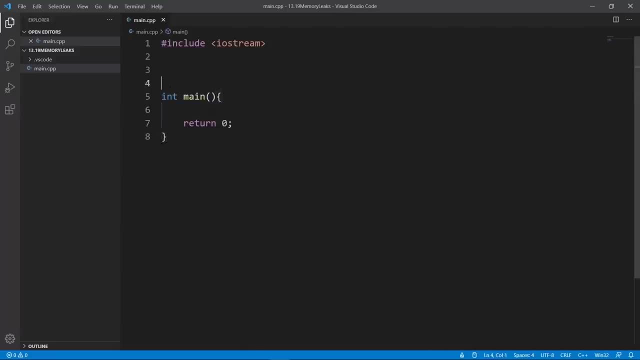 this in Visual Studio code. we are going to clean this up a little bit. bring this up here. we have a variable called p number. it is a pointer to ant and we initialize that with the address of a piece of memory that is allocated dynamically. on the heap we store a 67. 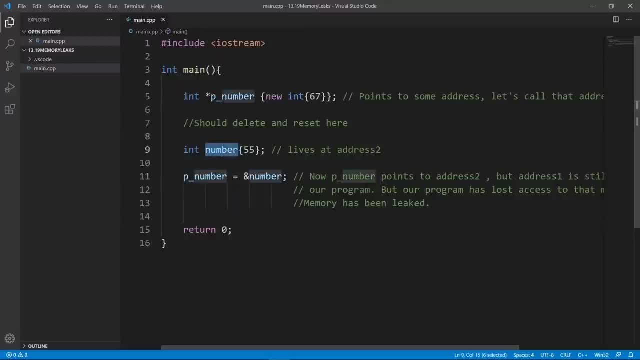 side and here down, you see, we set up another variable on the stack. again, this is a stack variable. it lives on the snack, it's not on the heap, and we take the address of this thing and assign that to our pointer here. the moment we do that, we have no more way we can access this dynamic. 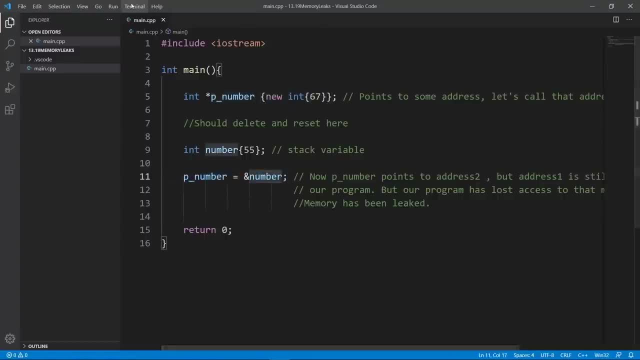 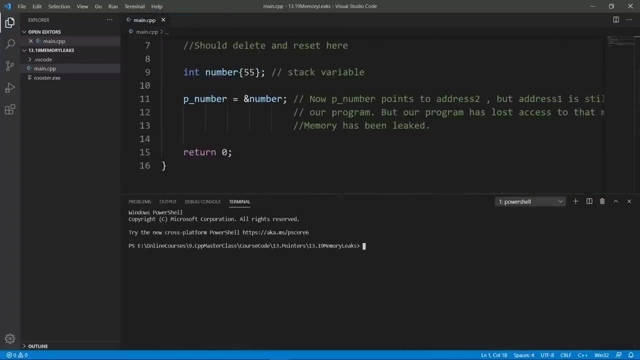 memory and we have leaked it, and this is really bad. the thing is, this program is going to compile. I don't think compilers have a way to stop you from making mistakes like this, so you really have to be careful and make sure that you are not leaking memory in your program. so if we run this program, 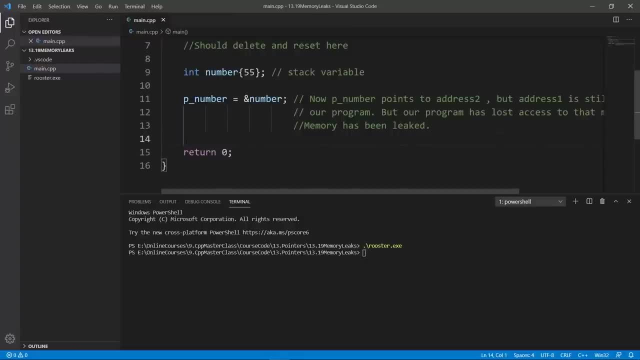 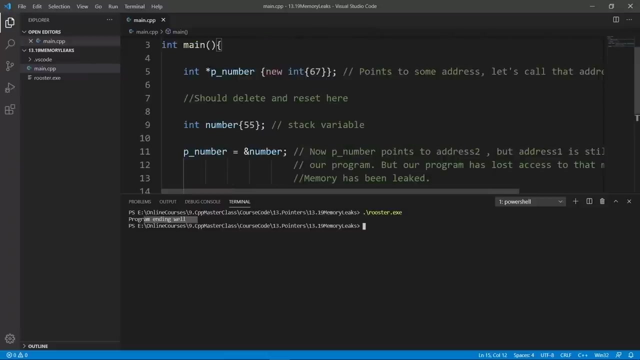 it's going to run. it's going to run and finish. let's say that it is ending well. okay, so we're going to build and see this run, the world is good so we can clear and run rooster and we're going to see that the program is ending well. but we are leaking memory here because the dynamically piece. 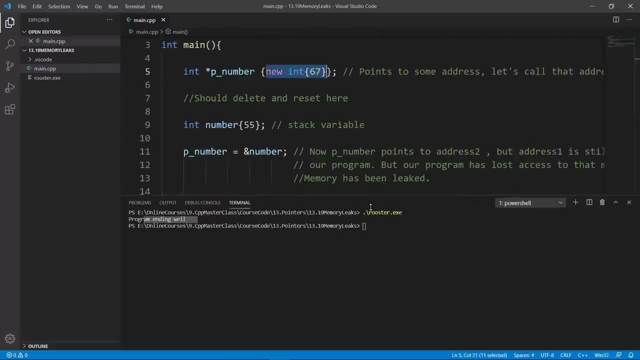 of memory that we allocated here wasn't released to the system, and when we did the assignment here we just lost access to it. so the operating system is going to thank. this memory belongs to this program that is ours here, but your program is either not going to be using this piece. 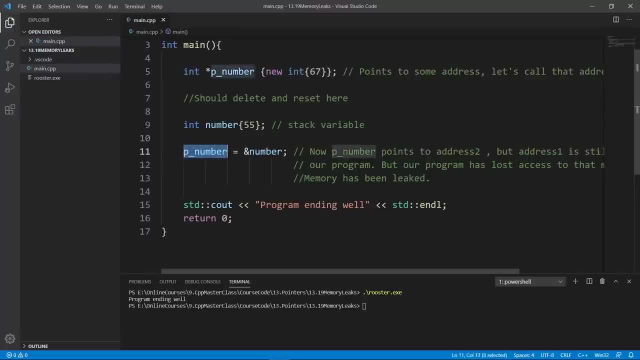 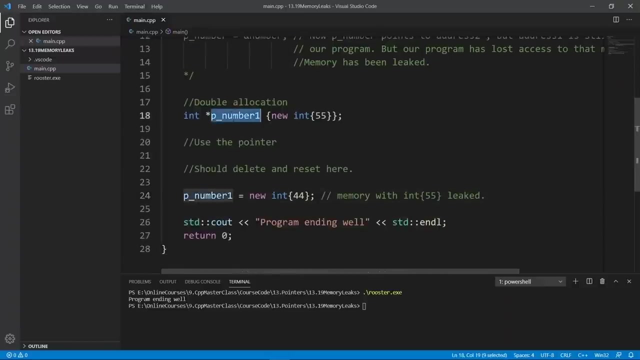 of memory because we have just lost the key that would allow us to go and do something useful with this memory here. so this is something bad and you should avoid it. the second example of memory leaks is when you do double allocation on a pointer. for example, let's say that we are using this pointer again and we are going to make this point to an address. 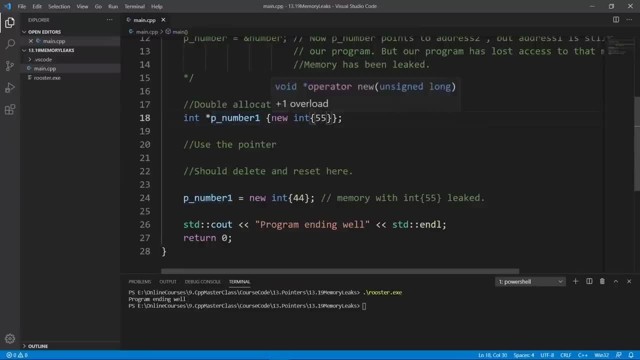 of a piece of memory that was allocated dynamically on the heap. the value inside is going to be 55, but we are using this pointer again to make it point to a new piece of memory containing the address of a newly allocated piece of memory on the stack on the heap. I mean, and this is really bad because 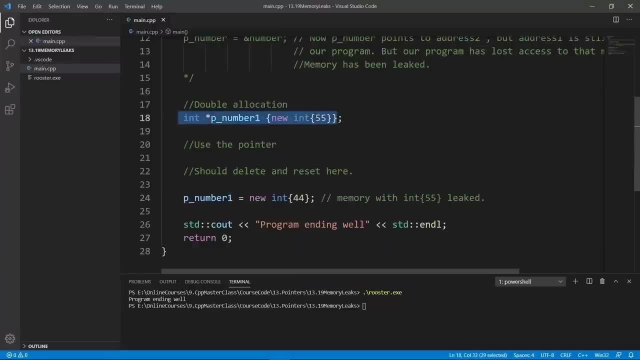 again. once we do this, we lose access to this memory here and it is leaked. the program here is not going to have access to it and the operating system is going to thank: we own this memory and it is going to be bad. and uh, down here maybe you can go and say: delete number one, P, number one, but this is not. 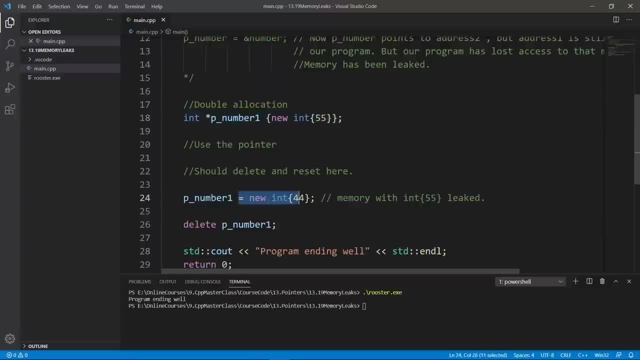 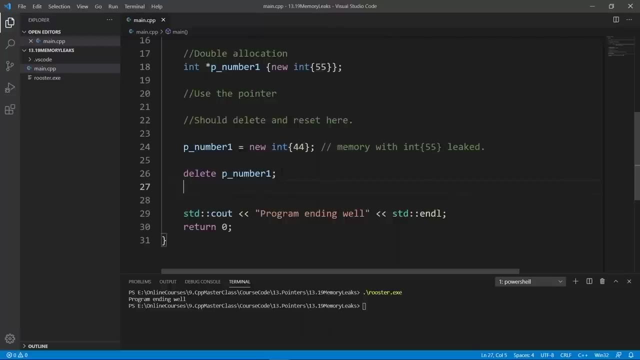 going to release the memory here. it is going to release the memory here with the 44 and the memory containing 55 here is going to be leaked. let's be good, C plus plus citizens and reset the pointers after we delete. so we're going to say: P number one equals no pointer and we are going 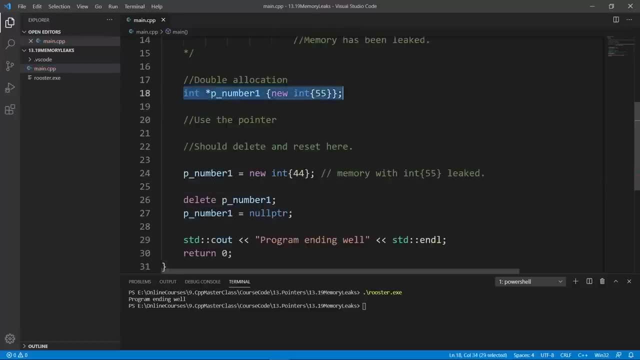 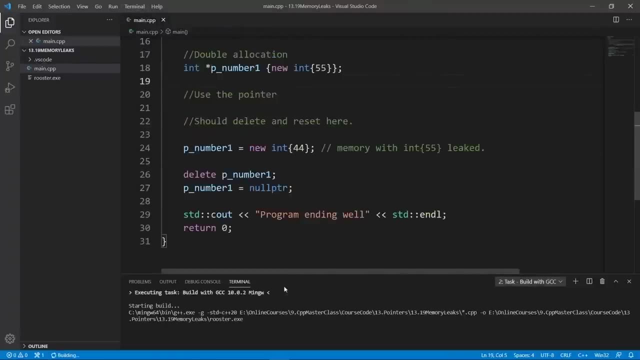 to be playing it safe here and again. we just leave the memory here and it is something you should avoid in your programs. if you run this program, it is going to run just fine. so let's see that, because I don't want to leave you with programs containing arrows if a run roaster again. 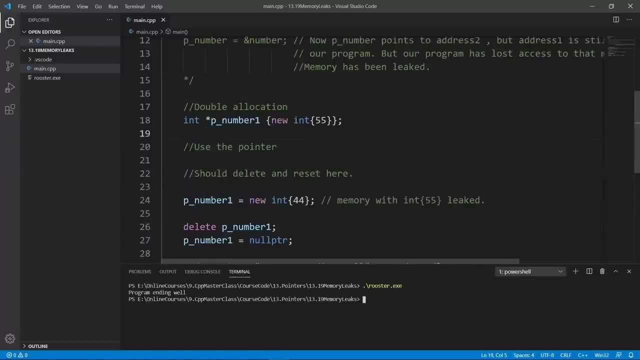 it's going to end well, but it is going to be leaking memory here, so we don't want to leak memory. avoid this like a plague. we're going to comment this out and show you that you can also leak memory when you have some nested scopes in your programs. okay, 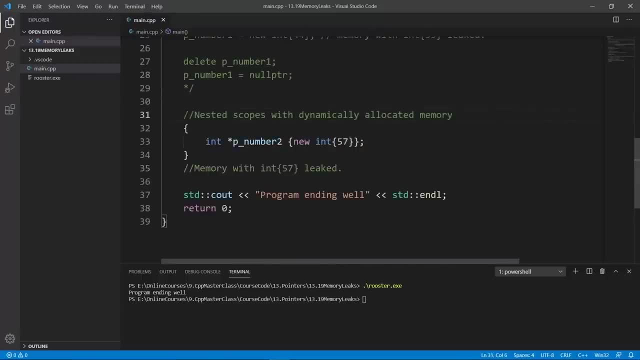 let's go down here and put that end. and here is a simple example: we have a nested scope, nested inside the main function and inside the scope. here we are setting up a new pointer and it is going to be pointing to dynamically allocated memory, and that memory is going to contain a 57.. 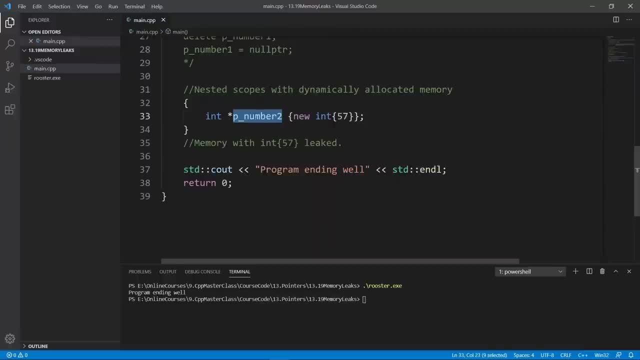 the only key we have to this dynamic memory is this P number two pointer here. but this P number two pointer leaves on the stack itself. so when the scope here is going to end, P number two is no longer going to be accessible and the memory is going to be leaked. if you really want to play, 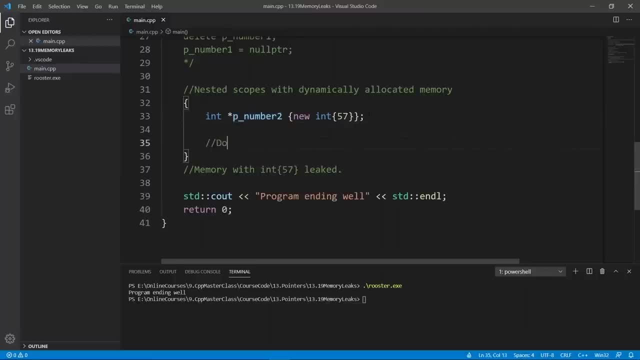 it safe. you can go do whatever you want with the dynamic memory and when you are done with that you can delete that piece of memory here while you still have access to P number two. but if you don't delete here in the scope where this thing was declared, if you hit the end of this scope, 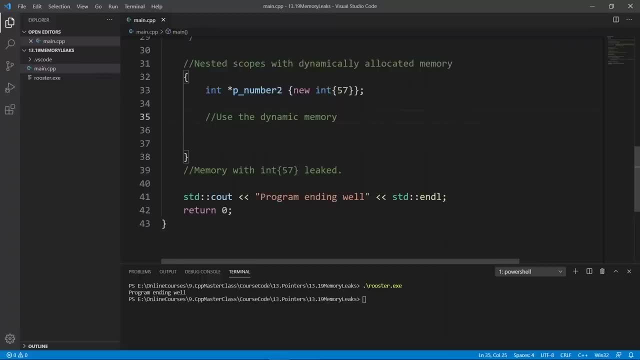 you're going to lose access to this pointer and you will be losing access to this dynamic piece of memory and you're going to be leaking memory because you're not deleting it. even if you want to delete it, you won't be able to do that because you don't have a key that is going to lead you to. 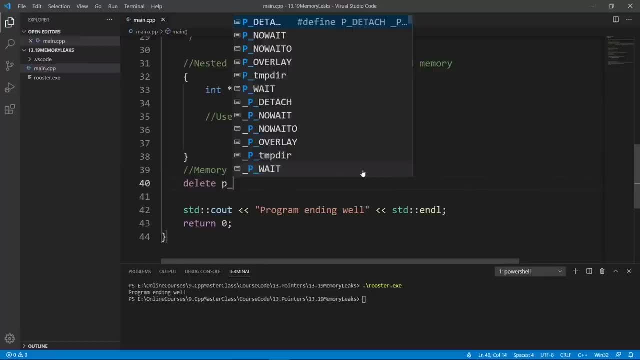 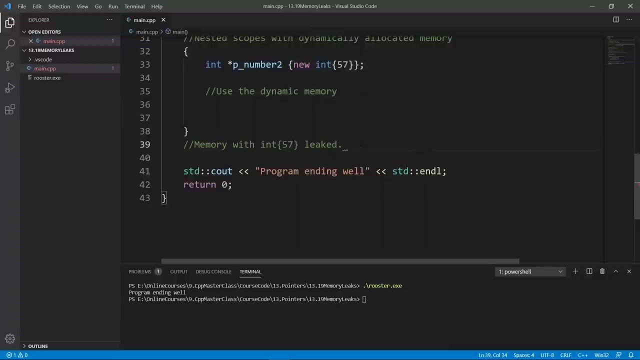 that dynamic memory. so if we try and do delete P number two here, this is not going to compile because we don't have access to P number two. P number two is scoped inside this nested scope here. this is what I mean. so be sure you are aware of this memory leak problem, the cases we have seen. 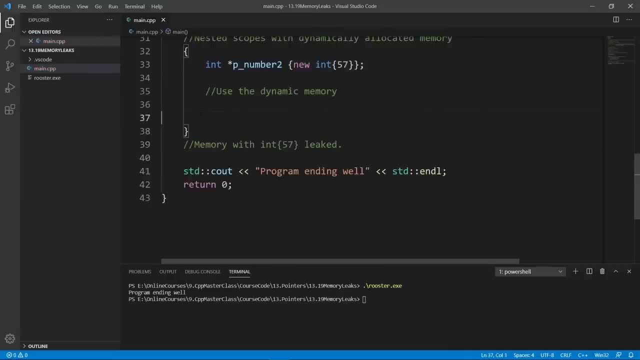 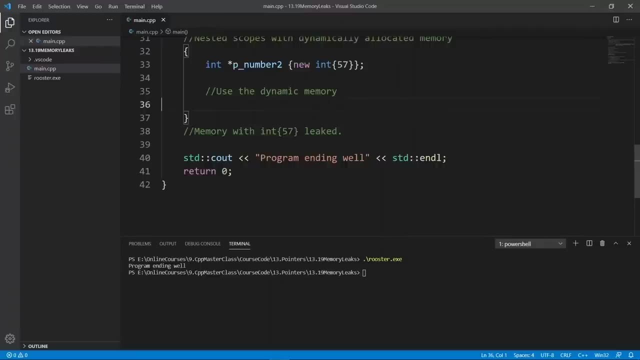 here are really extensive enough to give you an intuition on how this is bad, and you're going to be avoiding this new programs and you're going to be on your way to become a better C++ developer. this is really all we said start to do in this lecture. 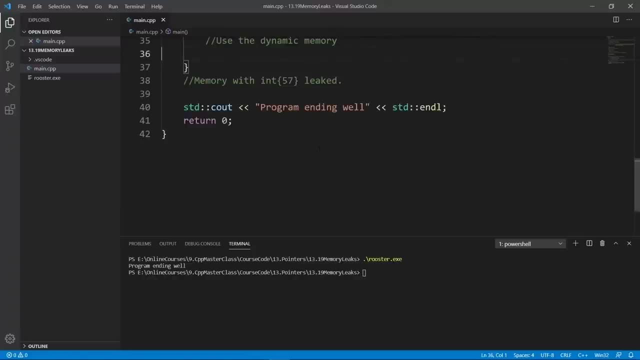 to learn about memory leaks. show you a few examples of them. I hope now you understand them. we are going to stop here in this lecture. in the next one we're going to learn about dynamically allocated arrays. go ahead and finish up here and meet me there. in this lecture we're going to look. 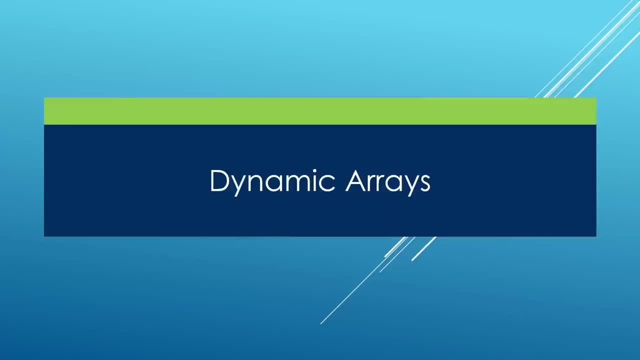 at dynamic arrays, and these are arrays you can allocate on the heap and they're not going to be stored on the stack. like we have seen before, the arrays we have learned about so far have been learned on the stack. we want to see how we can allocate arrays on the heap if we happen to need. 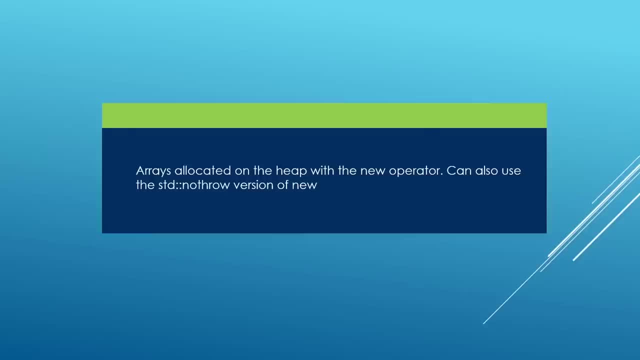 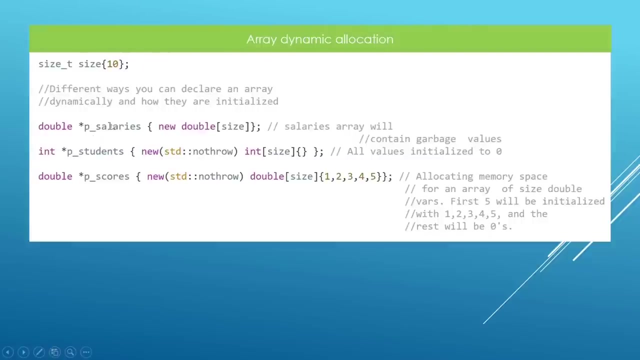 that in our applications arrays are allocated on the heap with the new operator. we can also use the std no throw version of the new operator if we don't want exceptions in our C++ programs. here is a simple example of how you can do that. we have a pointer called p salaries. it's going: 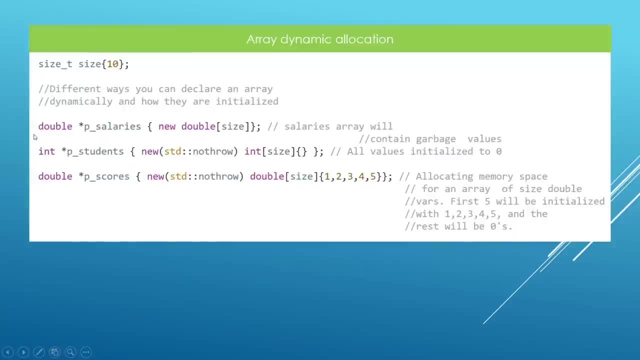 to be a pointer to double, and it is going to contain the address to the dynamic memory that we allocate on the heap, which is going to contain an array of doubles of this size here. okay, this is an array that is going to be initialized with junk values, because we are not 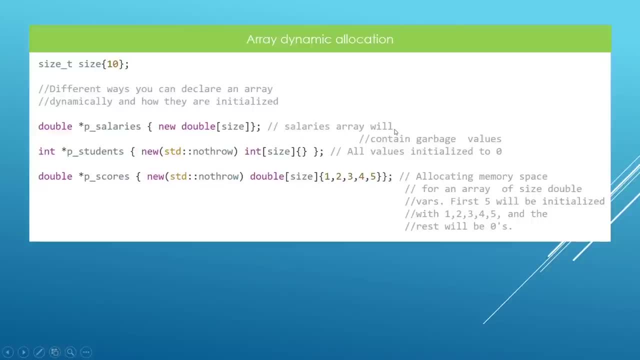 initializing that explicitly. so this is something you need to be aware of. okay, p students is also going to be containing the address of an array that is going to be allocated on the heap. we are going to call the name array. so if you are using a whole array in p fell, you chooseize. 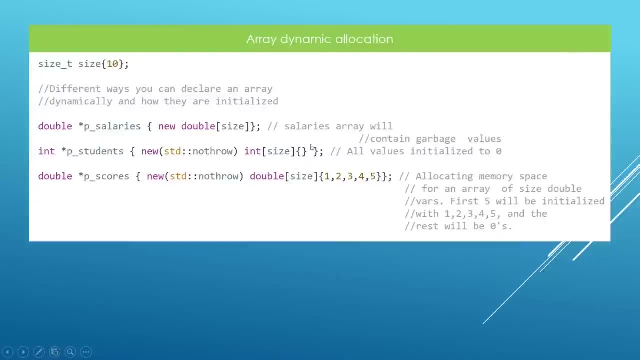 only on the heap and then, when you call it, you can select allt. i went in and you can Tell me for the first time that the values inside his array will be initialized. result is going to be initialized V to zero instead of zO. all the values inside are going to be initialized to. 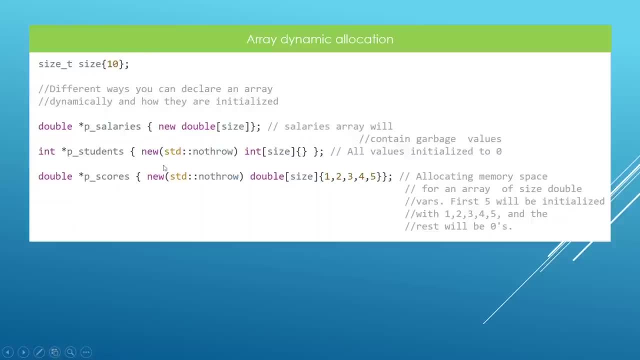 zero. this is what we mean here. we also have a p scores array. we are using the sd no throw version of new and it is going to be this size and initialized with one, two, three, four, five. okay, if that is the case, if we are looking to divide our factors, s t max to welcome or drop guys. 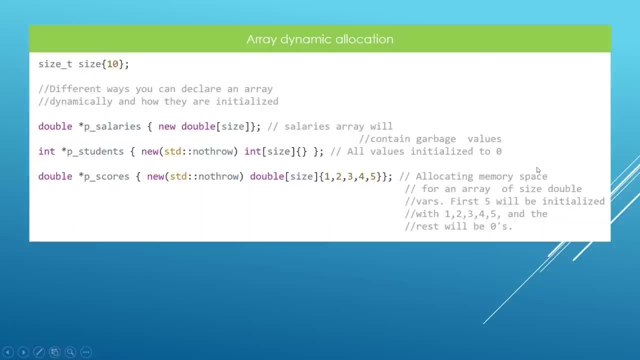 okay, if the array is a littlerous, then we're going to explain that part of the argument at this point. that s? t max is the state of size other. why is that initialized? because when we are using formal is bigger than five. the remaining slots are going to be initialized with zeros, just like we saw with 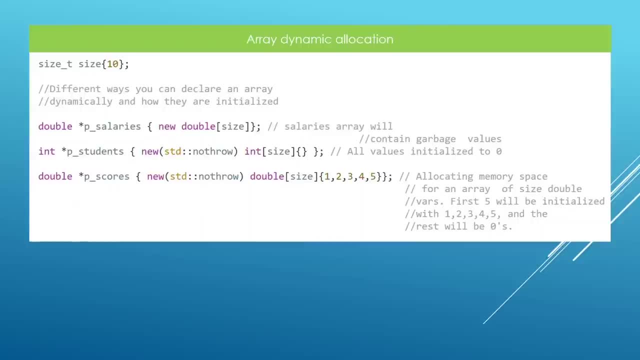 the arrays we have learned about previously that were stored on the stack. this is really how you work with these things and i hope it is super clear. again, we are calling the new operator this is going to allocate. however, memory space is needed to store these things on the heap. 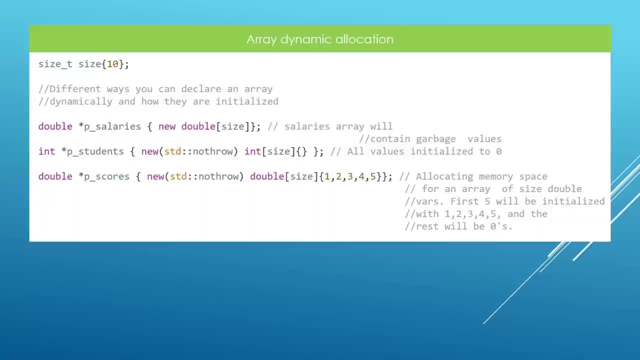 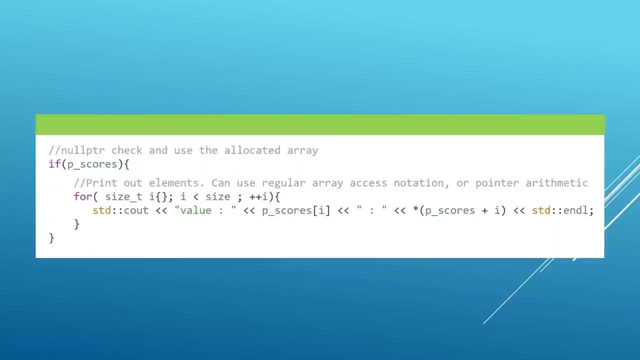 so if this array is going to contain 10 elements, we're going to allocate enough space to contain 10 double elements on the heap and we're going to be pointing to that with the p salaries pointer. that's what we mean here. once you have your dynamic array allocated on the heap, you can try. 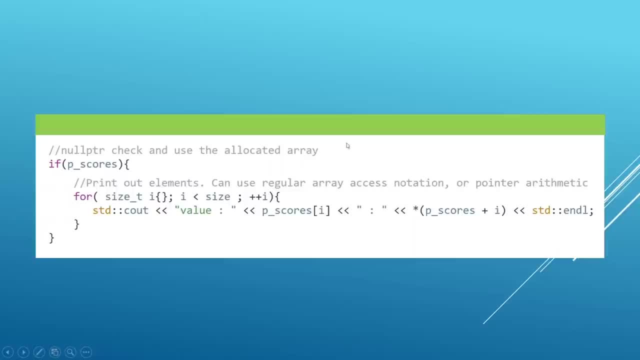 to do things with it. for example, we can try and loop through the scores and print them out. here you see that we are using the angle bracket syntax and the pointer arithmetic syntax. it is going to work equally well. you can choose whatever you want, but i just wanted you to see that you can use both. 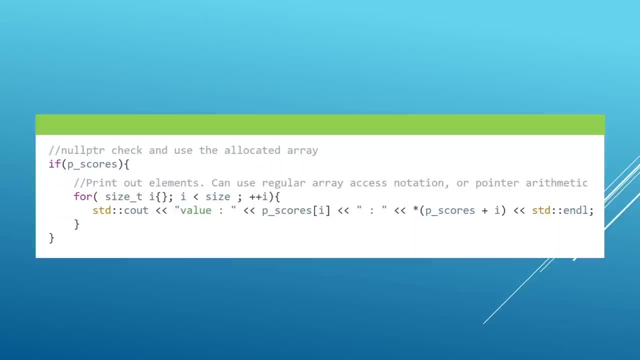 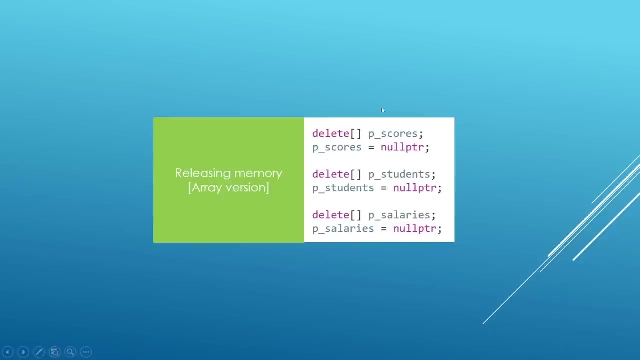 versions here. the next logical thing to think about when you talk about dynamic memory allocation is how you release the memory to the operating system when you're no longer using it. and this is the syntax to do it with arrays. you say delete, you put angle brackets and you say the pointer that was used to. 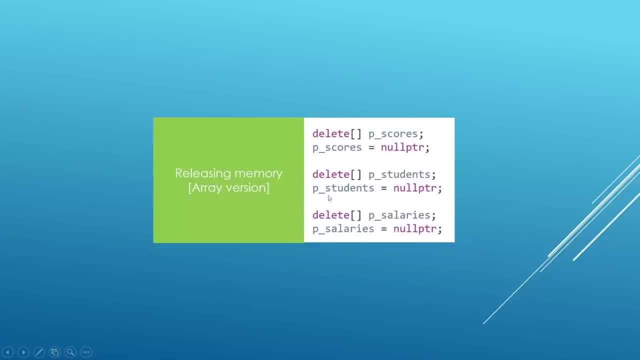 allocate that memory in the first place, and after you do that, you have to remember to reset the pointer to no pointer because you are a good c++ citizen. and this is really all we had to say in this lecture. this is how you dynamically allocate arrays on the heap before we head. 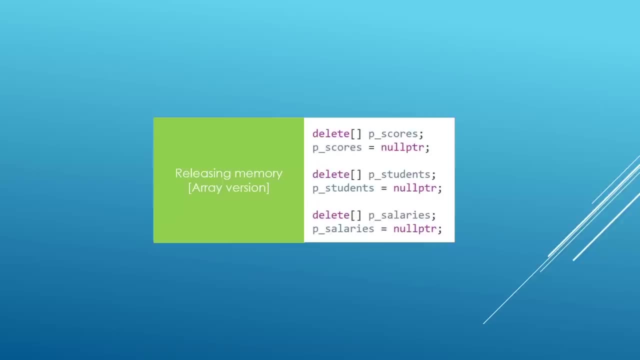 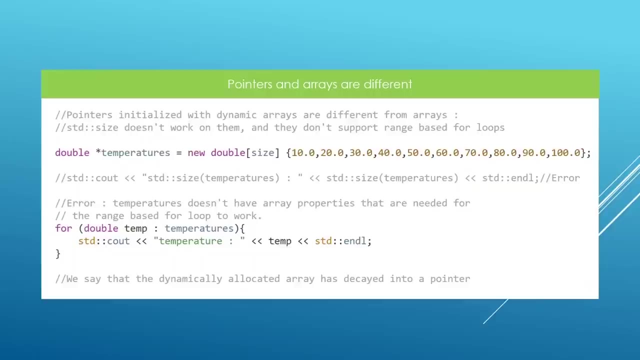 over to visual studio code and play with this, though i want you to keep in your mind that arrays you allocate dynamically on the heap are very different from the arrays that we have learned about before, and that's because they don't work with std size, and they don't work. 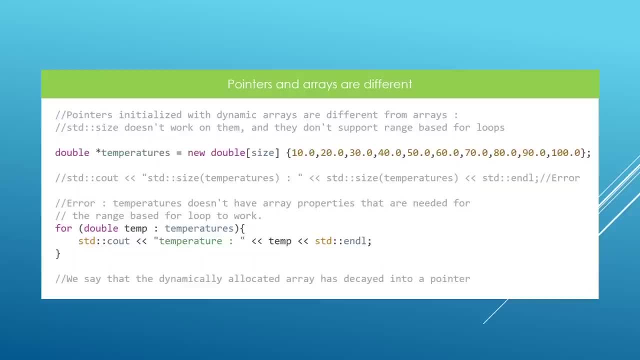 for range based for loops, and that the reason for all these limitations is that when you do something like this, the array really decays into a pointer and it loses information that would otherwise be used to deduce the size, that is used by std size and there are other things that are used by the 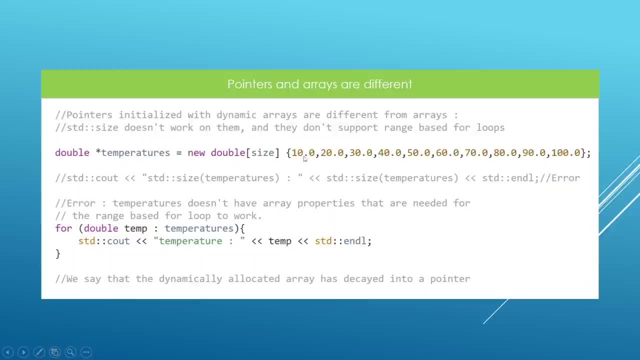 range based for loop that they lose when you store and refer to them using a pointer like this. that's why we have this limitation. keep this in mind. if you are using a dynamically allocated array on the heap, you're going to be using other techniques to deduce its size. 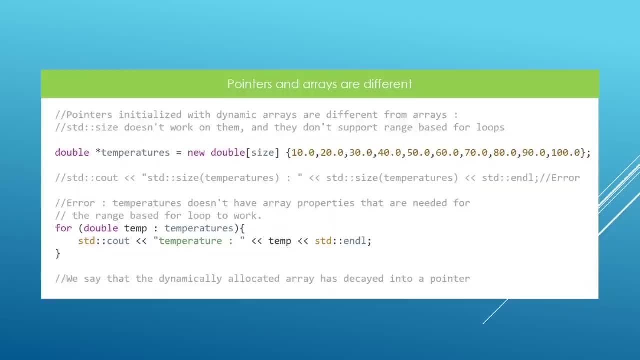 and it is not going to work with a range based for loop, so we will have to use other kinds of loops that we have learned about in this course, and it is going to work pretty well. this is really all i had to share in this lecture. now i think it's time we went to visual studio code and actually 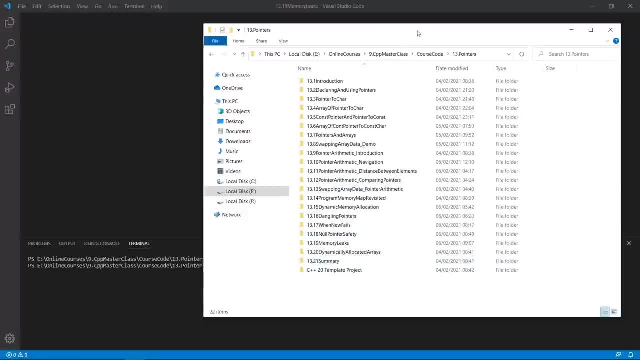 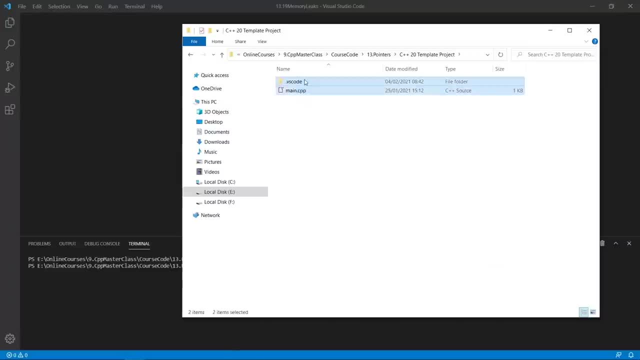 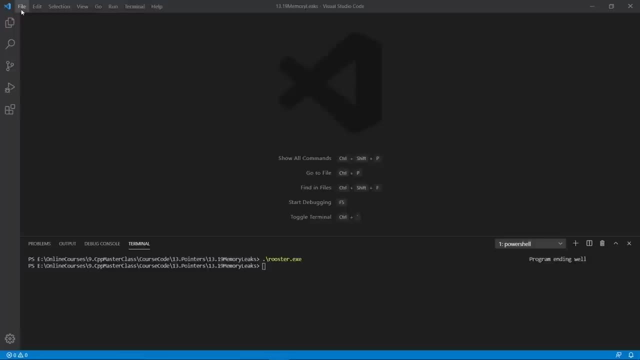 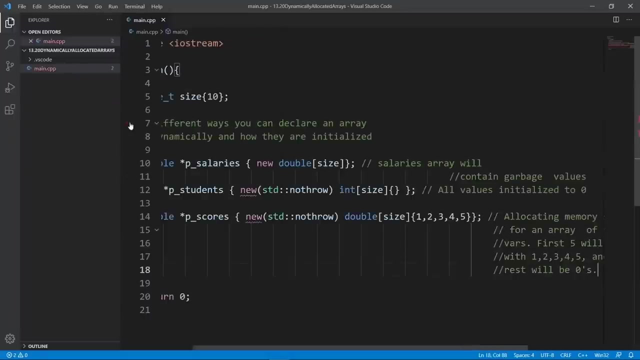 tried this out. here we are in our working folder. the current project is dynamically allocated arrays. we are going to grab our template files and put them in place and we're going to put that in the current project and open this in visual studio code, like we always do, and we are going to go down and put in some starter code we can play with here. 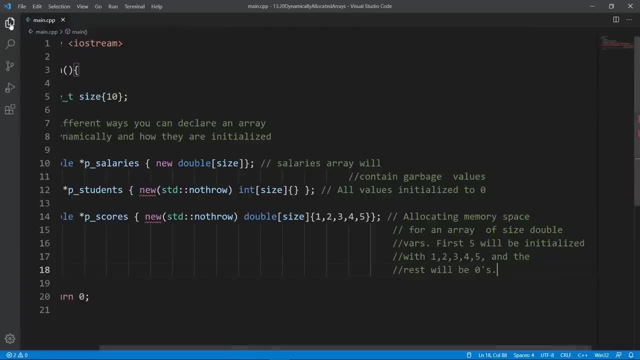 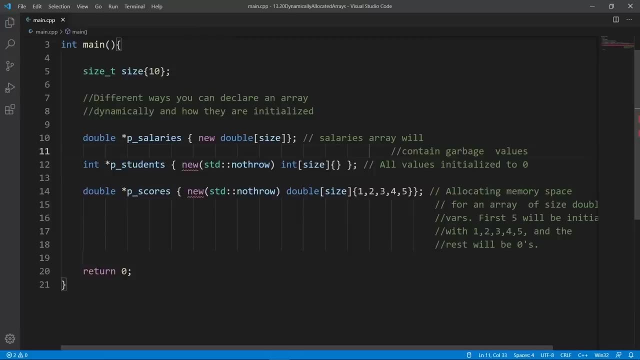 we're going to click on this file icon to remove this pane and we're going to try and show the code here and again. you see that visual studio code is freaking out when it sees the std no throw version of the new operator here. but it is going to work when we hit the compiler. okay, let's. 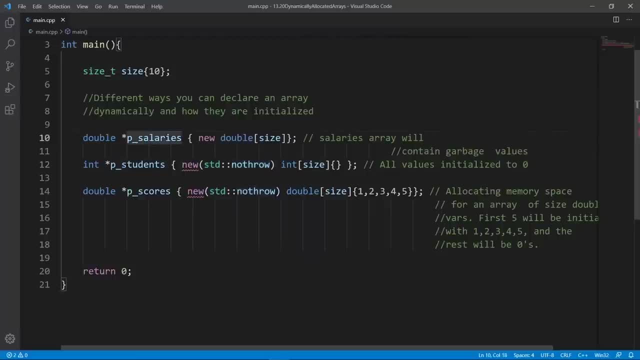 get to the context of this part, let's go ahead and explain what we're going to do in the next lecture. okay, so we are allocating three arrays on the heap dynamically and we are going to be storing the addresses to these arrays and these pointers. for example, pcellarese is going to store. 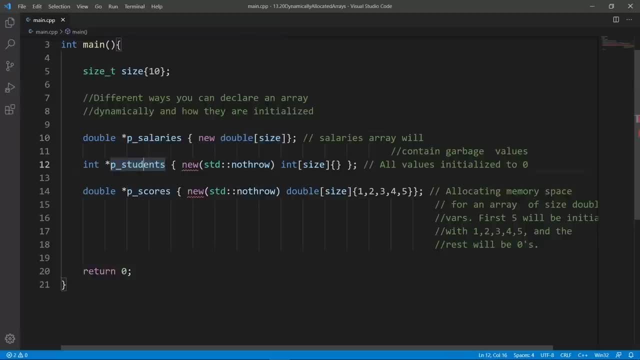 the address to this dynamic array which is going to be living on the heap, and it is going to be the same case for p students here and p scores. i don't think there is much to explain here, because we have already learned about arrays. we know about the size of an array. 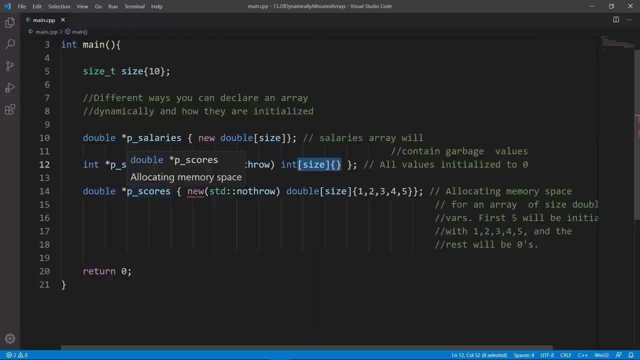 memory location that is going to be storing variables of the same type. this is really what we're going to have, so let's try and compile this and see that it actually goes through our gcc compiler and it is going to work fine. and another thing you should notice is that this is really 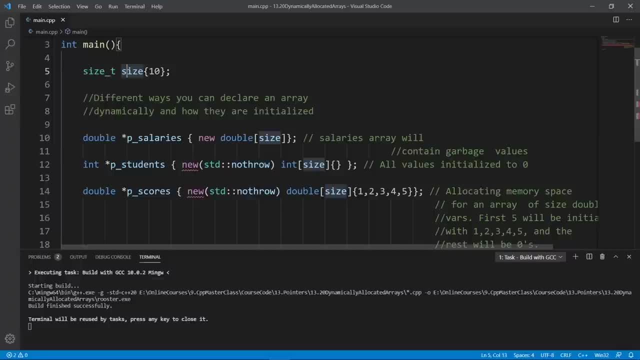 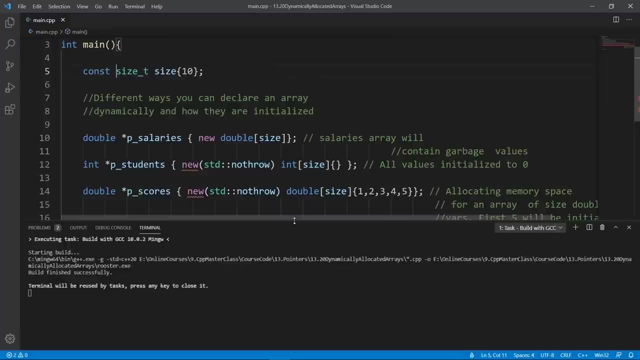 compiling even if what we are using to store the size of the array is not const. remember, for stack arrays or static arrays that we had on the stack, we had to make sure this guy here is const. okay, that was a requirement and if you didn't fulfill that, your code wouldn't compile. now you 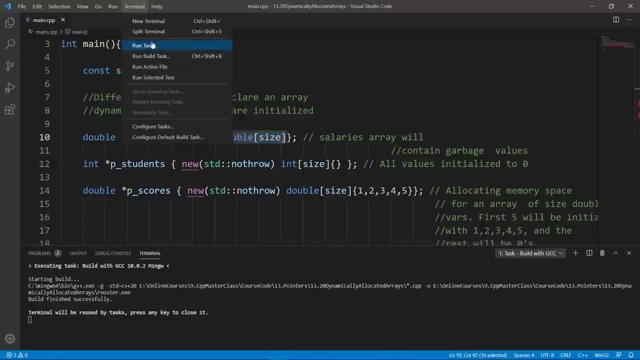 see that with dynamic arrays, the code is actually compiling, even if it's not const, and this is something you should be aware of. let's build this again. i just messed up my things here and the build is good if we go down and run it. we're not. 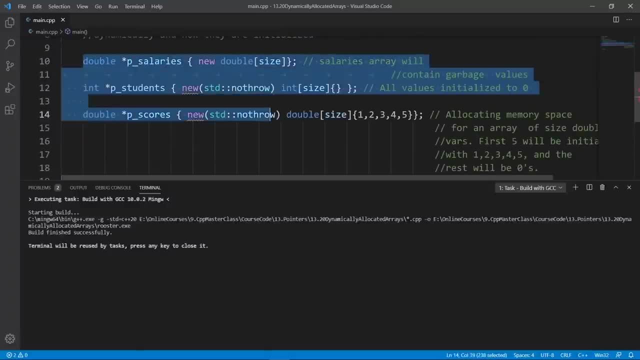 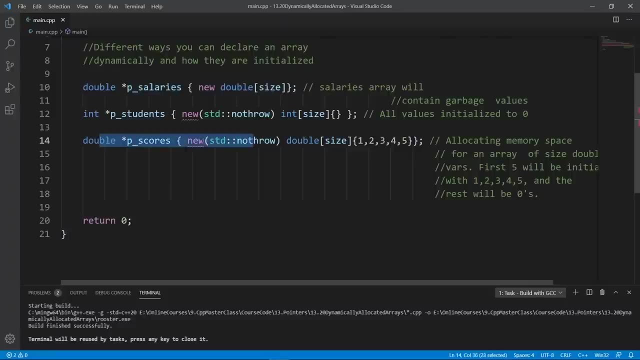 going to be able to run it. we're not going to be able to run it. we're not going to run it to see anything, really, because we're not having any output in this program. but this is how you can allocate space for a dynamic array on the heap. now let's try and print some of the data in this. 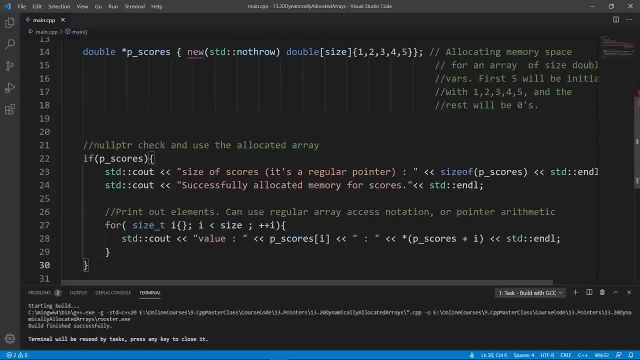 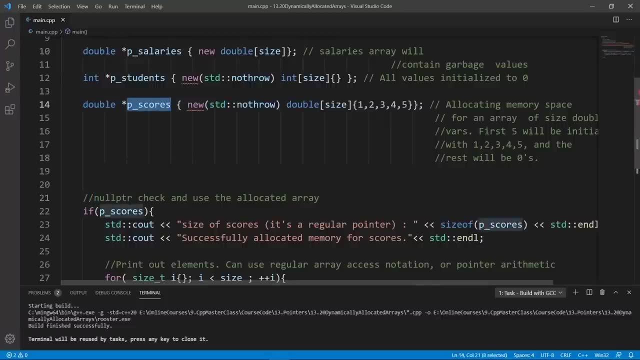 course here. let's go down here and actually do that. we are going to do a null pointer check because we want to make sure that memory was actually allocated for the p scores array, and after we do that we're going to look for size times and we're going to 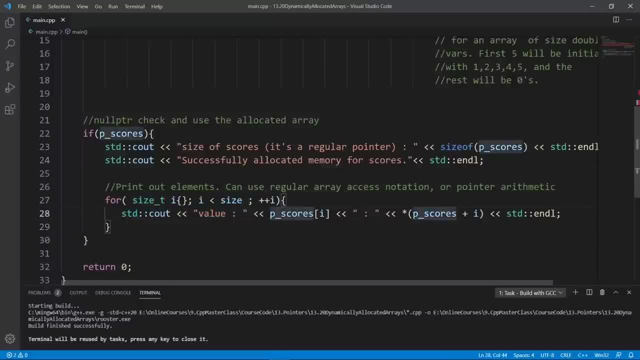 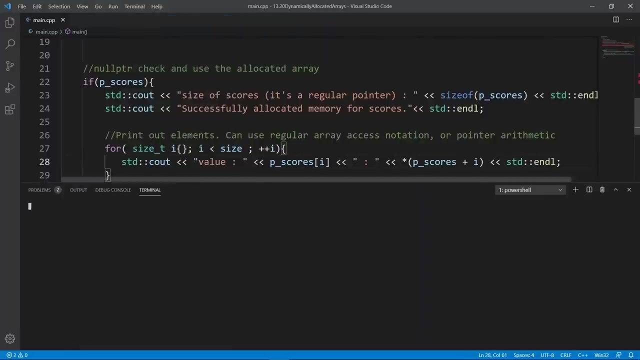 be printing whatever element is at each iteration, the index at each iteration, and you see that we can either use the angle brackets notation or the pointer arithmetic notation. it is going to work equally well. if we weld this, let's bring up our terminal. we haven't opened one and let's go down. 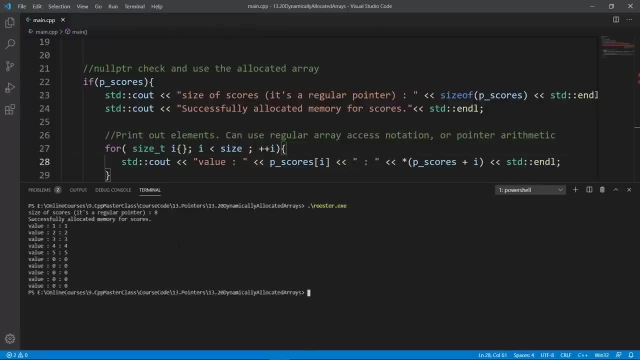 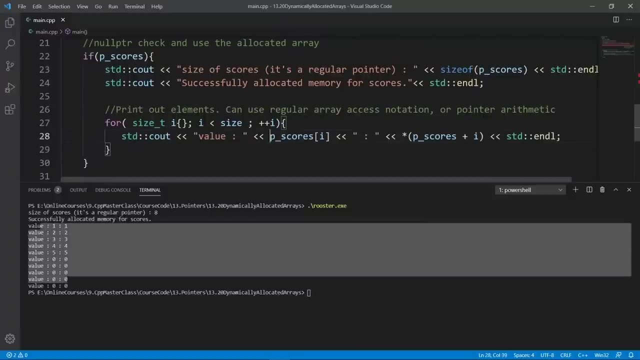 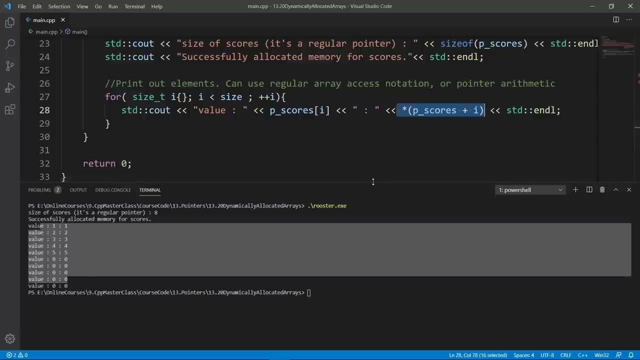 and clear and run rooster. you're going to see that successfully allocated memory for scores and we're going to be printing the data, first using the angle brackets notation, second using pointer arithmetic, and you see that it is working pretty well. one thing you should have noticed now: 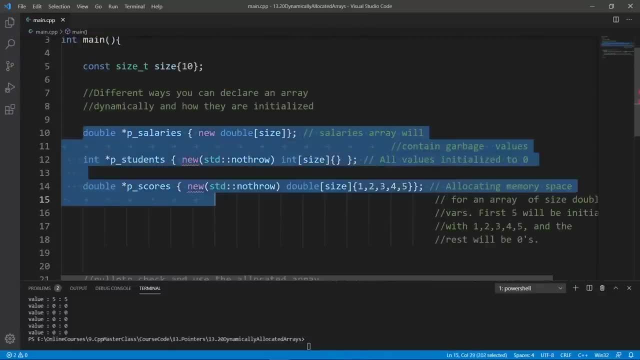 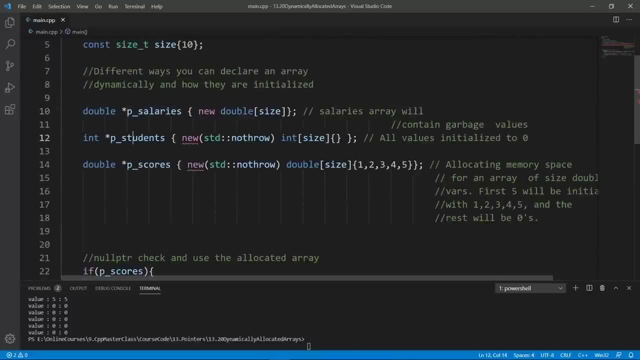 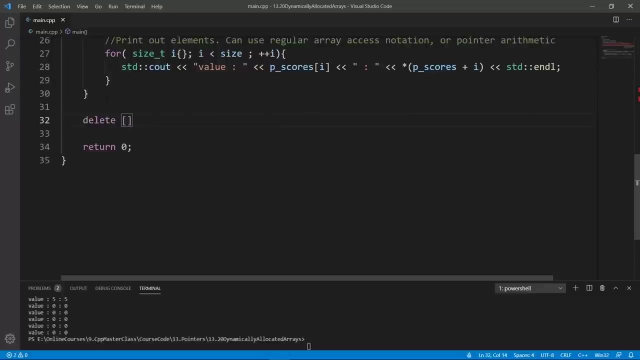 is that we haven't actually released the memory that we have allocated here, and this is something really bad. so we're going to see how we can do that. we have allocated space for salaries, p students and scores, so let's go down and do that and we're going to say delete and we're going to have anger. 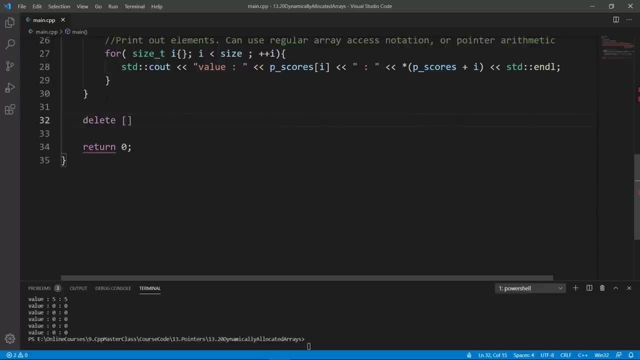 brackets, because this is an array we are releasing memory for, or, to be exact, a dynamic array which was allocated on the heap. so we're going to say p salaries and we're going to reset that pointer to no pointer because we are good: c plus plus citizens. so we're going to do that, no pointer. 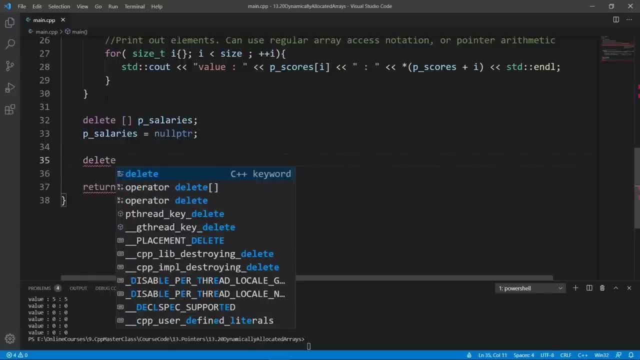 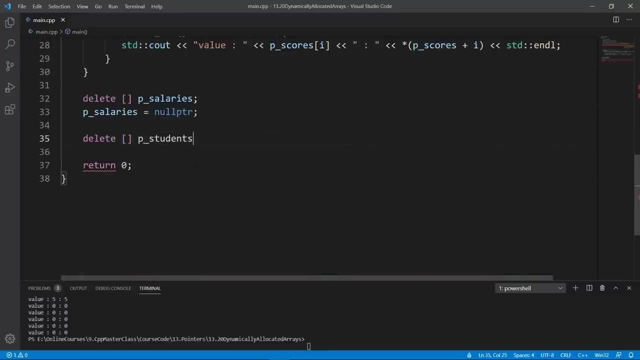 and we're going to do the same thing, delete. we are deleting space for a dynamic array, so the angle brackets here, the square brackets, i should say, and we are going to delete p students. i think yes. so we're going to say p students and we're going to say p students and we're going to reset this to no. 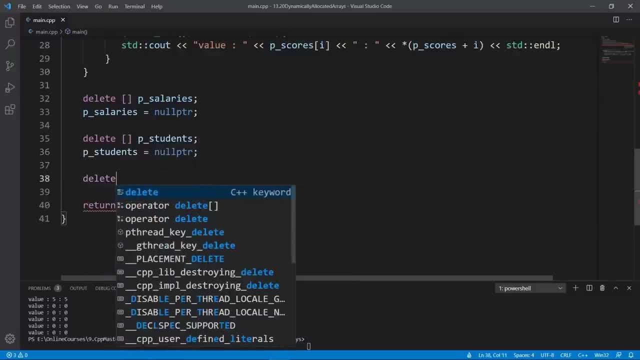 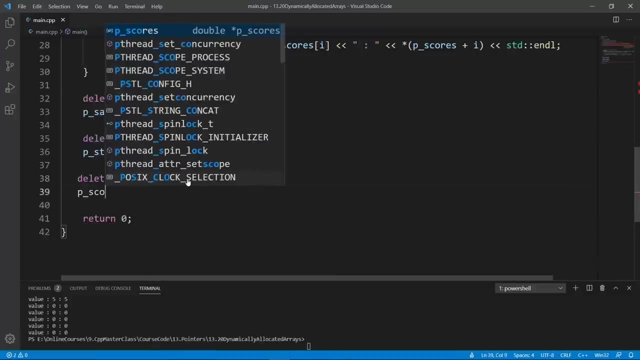 pointer and we're going to do the same for p scores. let's grab this here. that's what we want. no, that's not what we want. we're going to say delete and say square brackets ourselves and we're going to say p scores and we're going to release that and say p scores and reset this to. 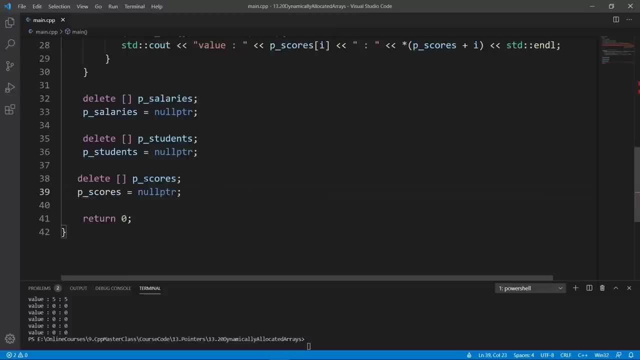 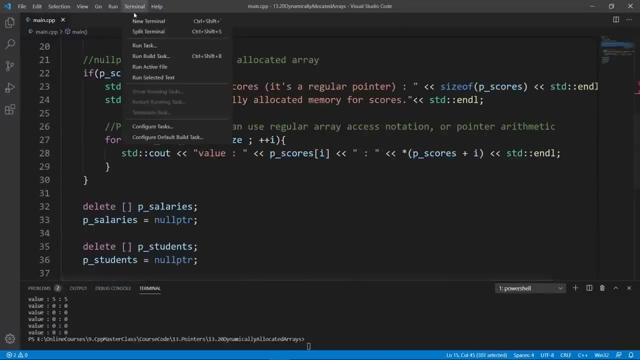 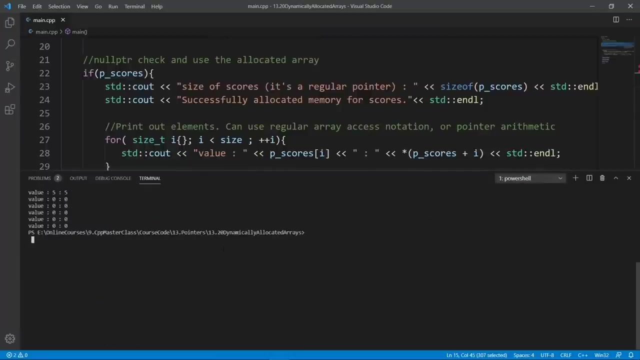 null pointer. now we are really playing it safe and our program is going to release the memory that we allocated in these three statements here. if we build the program, it is going to go through well. so we're going to build with gcc and we are going to clear and run rooster and it is going to. 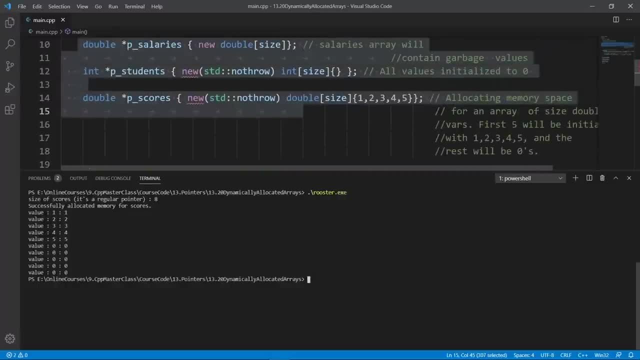 run pretty well. you see that it's going to run pretty well. you see that it's going to run pretty well. you see that for p scores we initialized the first five elements and the remaining elements were initialized implicitly by the compiler to zero, and you can see that here. i don't think i explained. 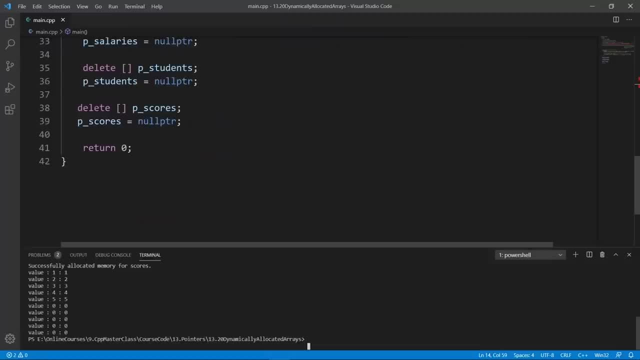 this, but this is my chance to explain this. i hope you understand. the next thing i wanted to explore before we close this video is the difference between static arrays and dynamic arrays. a static array is an array you allocate on the stack, like we have been doing before. 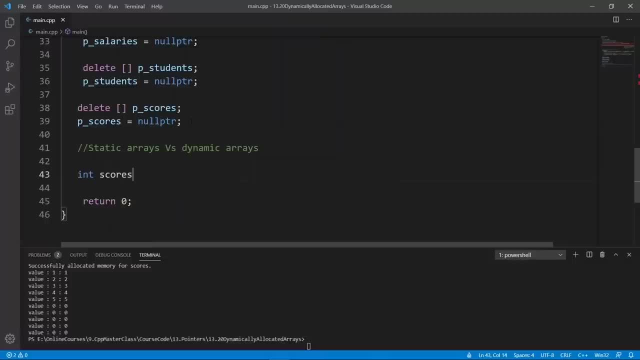 and you do it using a syntax like, let's say, scores- why not? and it is going to be an array. let's say it is going to contain 10 elements and we are going to put in our values in the format that we know, and we're going to go all. 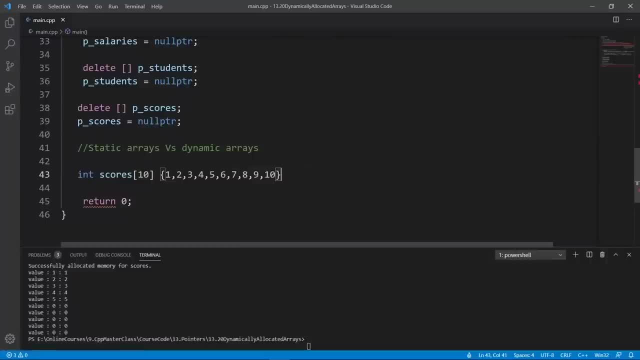 the way to 10. let's put in a 10 here and we're going to end this with a semicolon. this array is cool and you can loop through it. you can do all kinds of crazy things with it. but i am going to emphasize two differences we have with dynamic arrays. one is that this guy is going to work with. 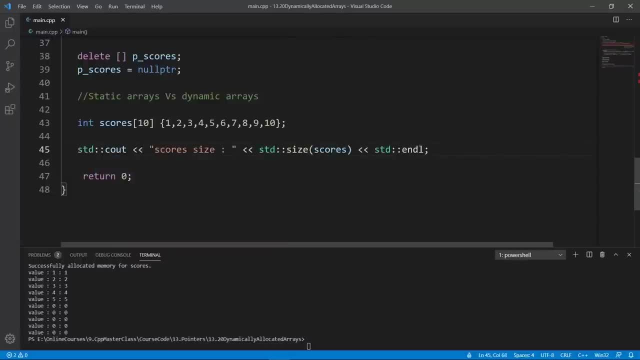 the size. so we're going to say c out, okay, this is going to work. if we compile this, we're going to get a good wealth- at least i hope. yes, the world is good. and if we run booster, we're going to get scores. size is 10.. the other thing is that you can use a range based for loop. 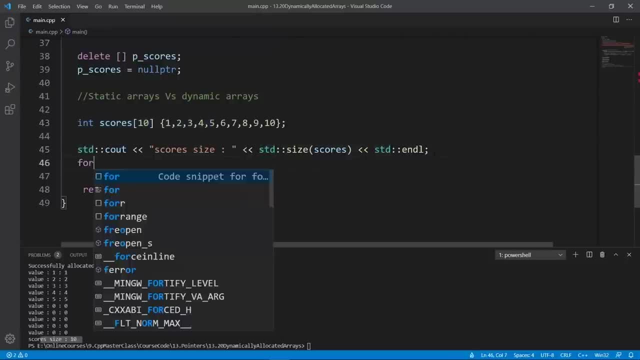 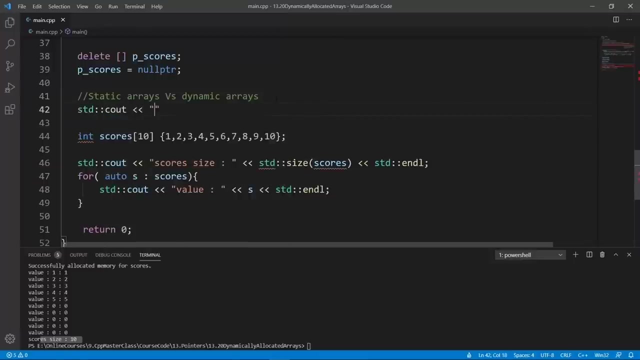 to loop through this guy here. so, for example, we can say for autumn score s, for score in scores, and it is going to work. so let's go down and say what we are doing here. or we can even say a single line to separate things here. i don't want to be confused, so i am going to do something like: 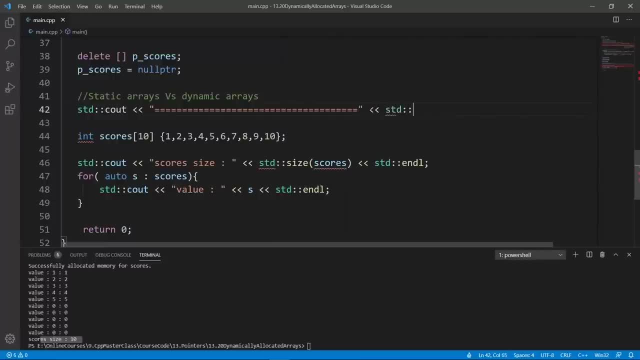 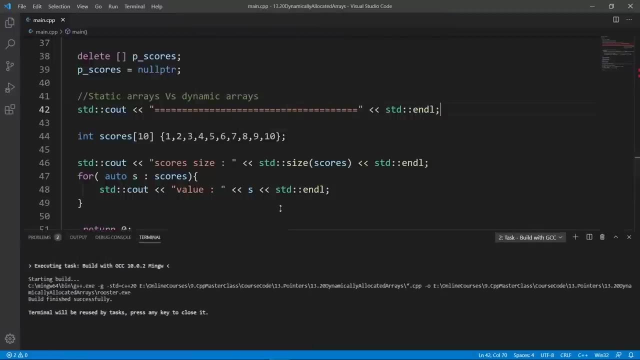 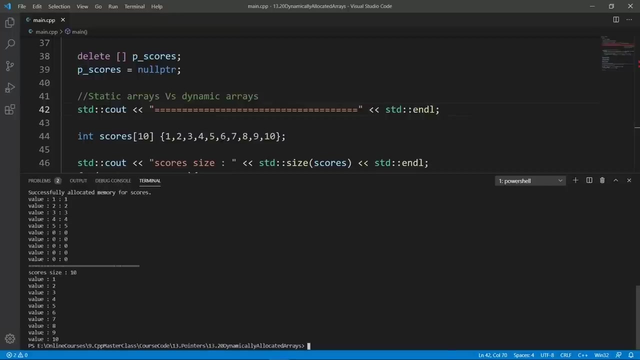 this so that i know where my output here is going to start. so i am going to build this with gcc. of course, the world is going to go through and if i clear and run rooster, i am going to see that the size is 10 and i am going to print my elements here. 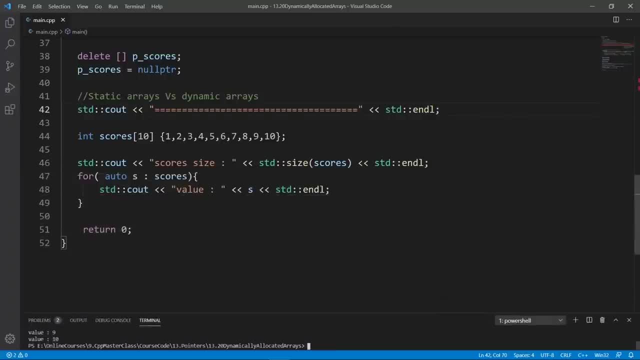 with a range based for a loop. okay, let's see how these things behave when we use a dynamic array. we are going to set up a similar array, but on the heap, which is going to leave on the heap. this array here is the static array in that it is going to leave on the stack. you have to be. 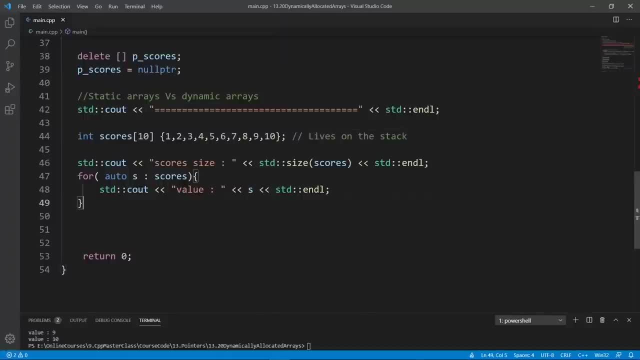 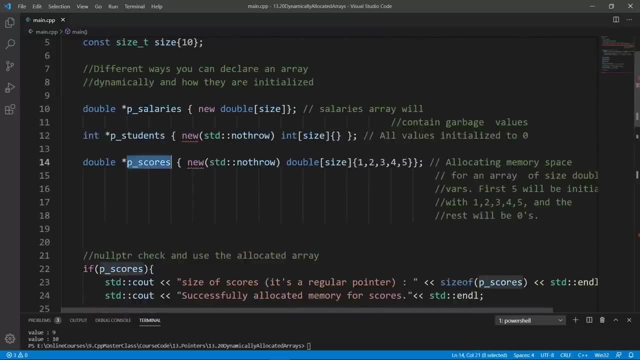 aware of these differences. okay, we're going to do another one, which is going to leave on the heap and the way we do that. we set up a static array and we set up a dynamic array and we set up a say endpointer, let's say pscores one, to make sure this is different from pscores that we have on top. 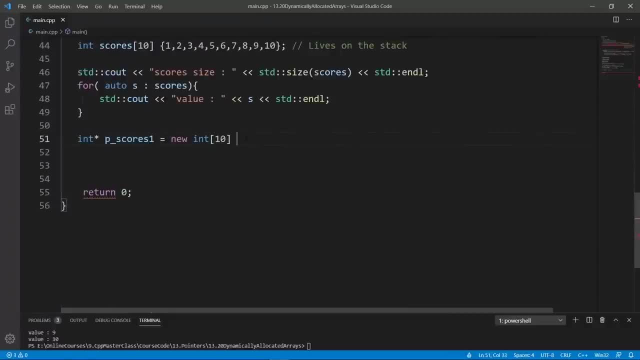 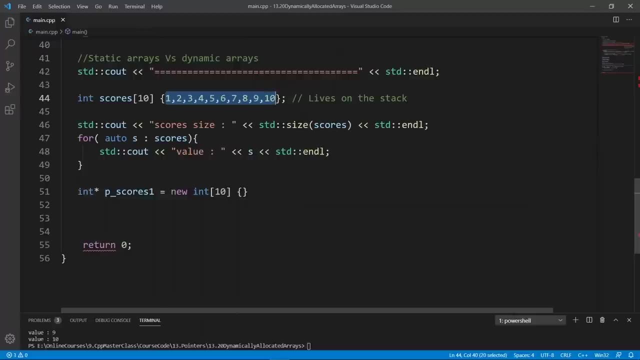 here and we're going to have 10 elements inside and we can even initialize this guy, exactly like we are doing here, but the data is not going to leave on the stack, the data is going to leave on the heap. if we do something like this, first let's make sure that the code compiles. we're going to 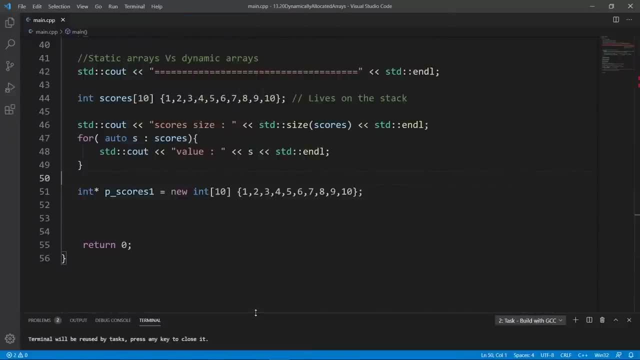 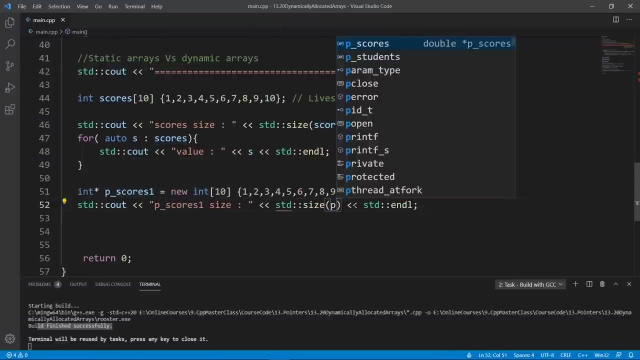 try and run this through gcc and watch the compiler output here. the build is good, so this is valid c++ code. we can try and use std size on that and we're going to go down and do that and if we do that we're going to say pscores- size, one size and say pscores if we try to pass this. 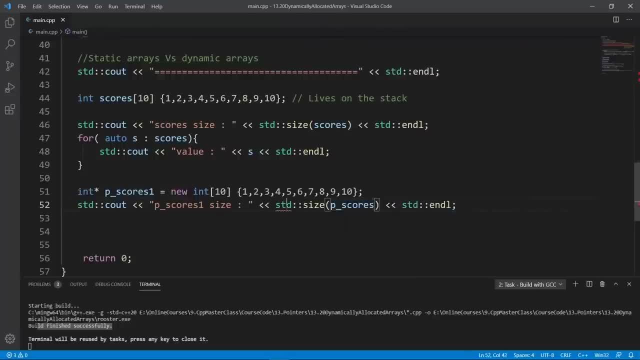 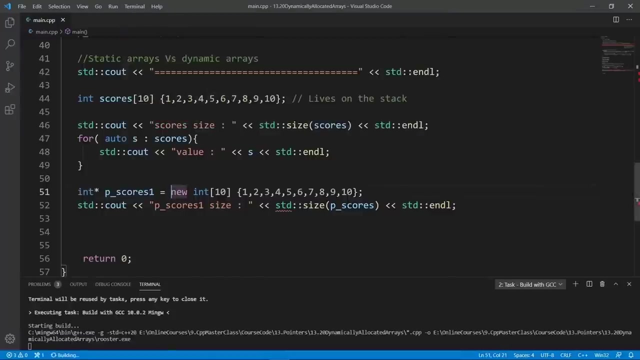 pointer. here you're going to see that visual studio code is going to freak out because this one work, the array here, has decayed into a pointer when we refer to it using a row pointer like this, so we can't really use it inside std size. so if we look at this, we're going to get a weird compiler. 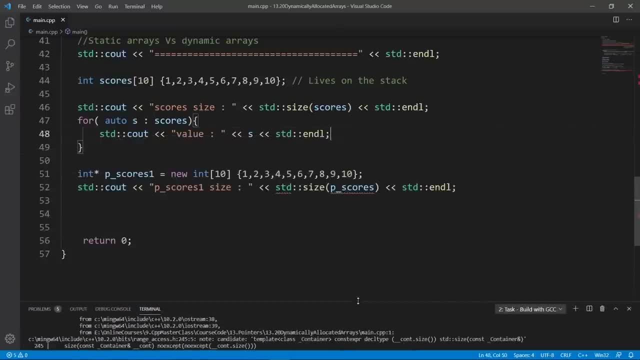 error, but this is going to be the problem here. okay, so you can't do this with dynamic arrays. this is one limitation. the other is that you can't use dynamic arrays like we are using a range. that's not going to work. so we're going to use dynamic arrays like we are using a range that's. 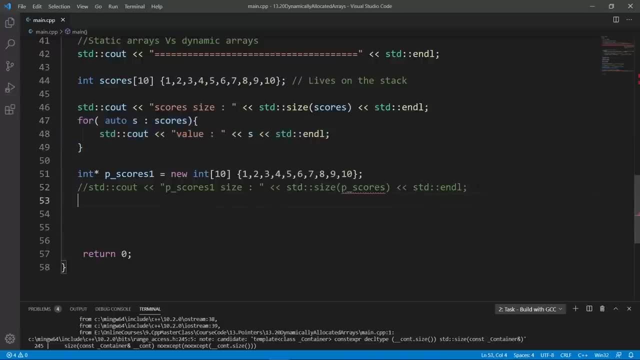 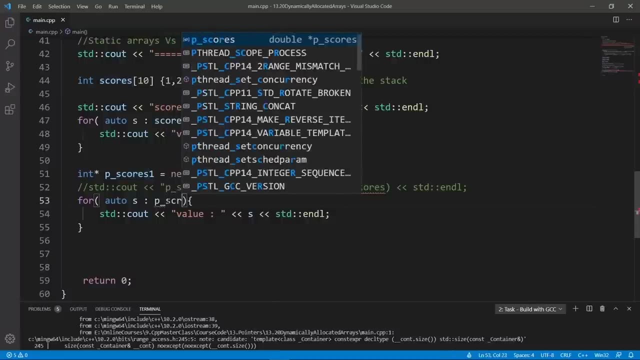 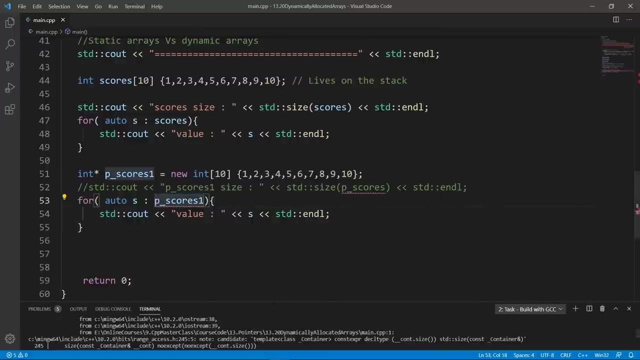 based for a loop here. so if we grab this loop and try to work with it on p-scores for example, this is something somebody might want to do- let's say p-scores one, okay, and try to print something inside, you're going to see that this is not going to work. the compiler. 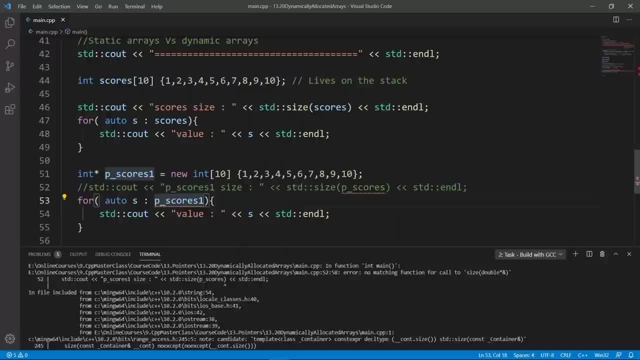 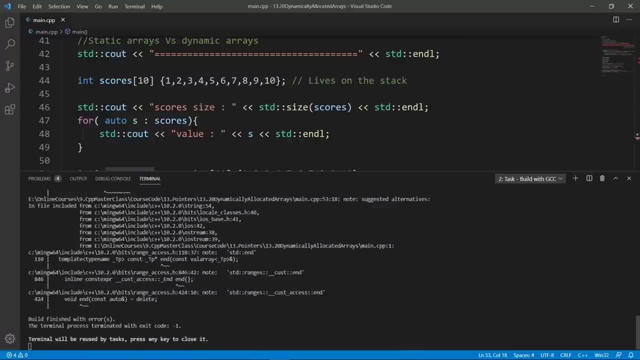 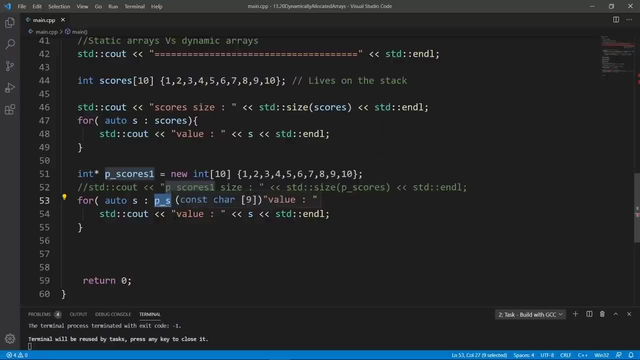 visual studio code is not going to like it first, and if we try and run this through gcc, we're also going to get a weird compiler error, and the problem is going to be that p-score is really not an array, it is just a pointer that is pointing to some location in memory. 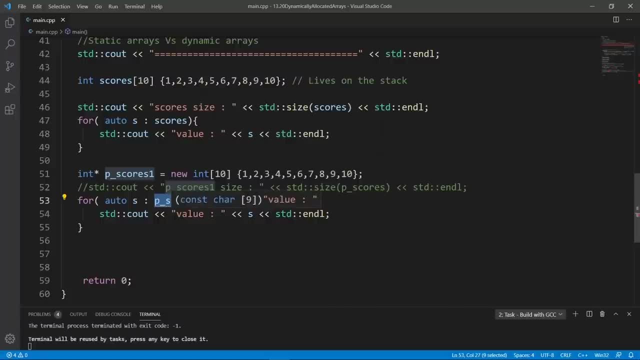 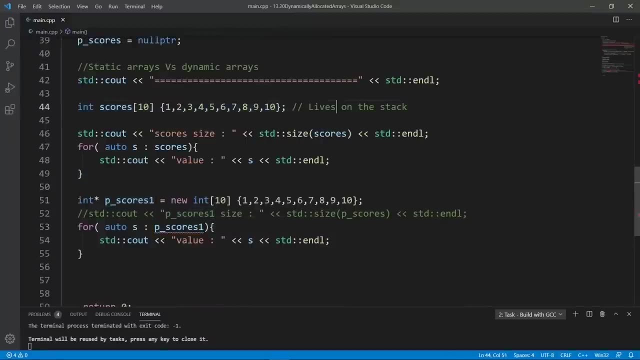 that's all it is and it doesn't have information that could be used otherwise to loop through elements like we can do for a real static array that is living on the stack. again, let's be super clear here and say that this array is going to leave on the heap. you have to understand these. 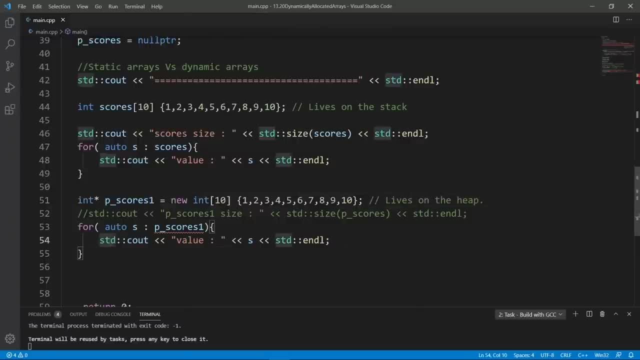 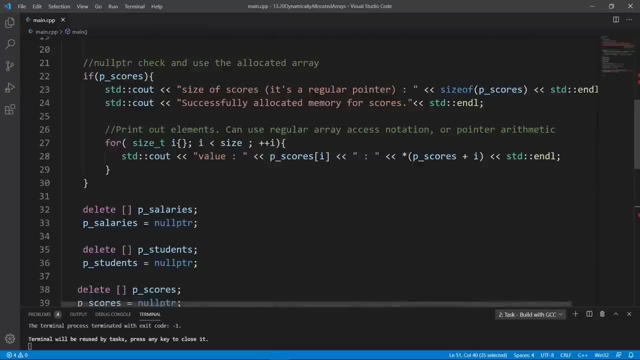 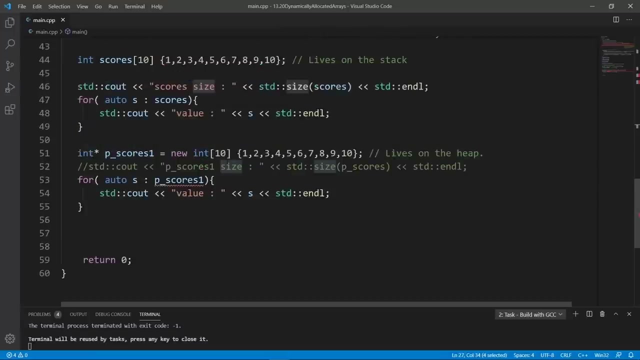 things. but this is really not the big limitation, because you can store the size of this guy in some variable and refer to it if you need that, and you can loop through the array exactly like we did here using size, and it is going to work pretty well. so don't be afraid to store your arrays on the heap if that's what you need in. 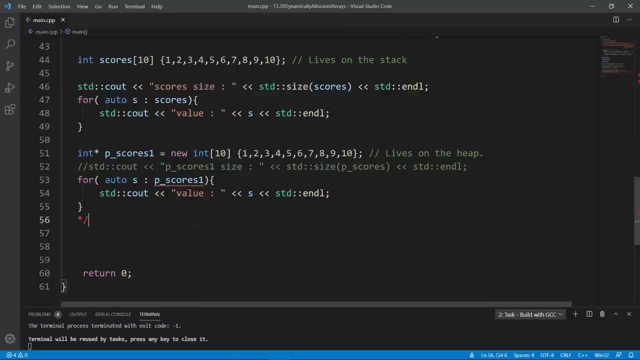 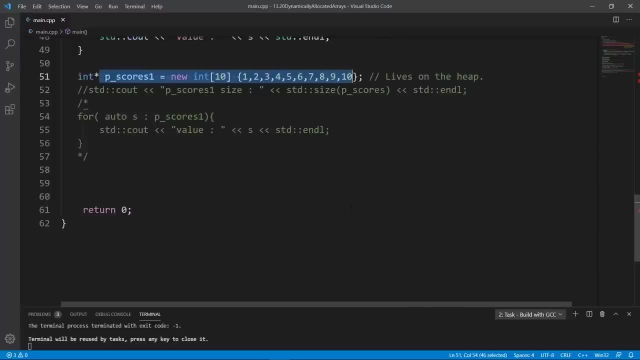 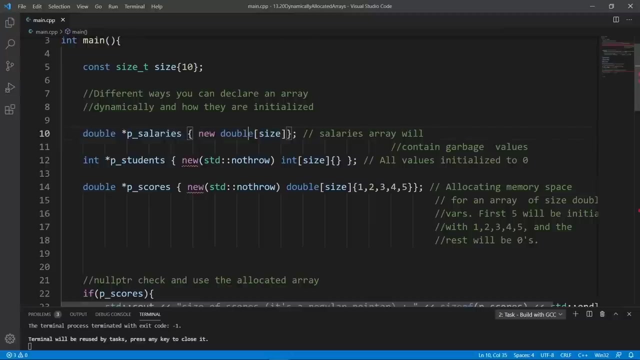 your application. it is going to work pretty well. you just have to be aware of some limitations that come with doing things this way here. this is really all we set out to do in this lecture. i hope you have a better idea about dynamic arrays. you set them up like this: the size here doesn't have 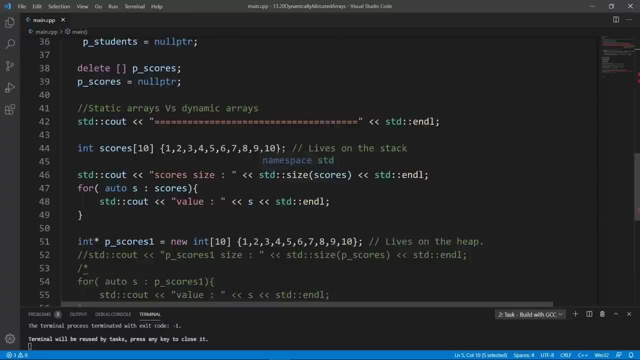 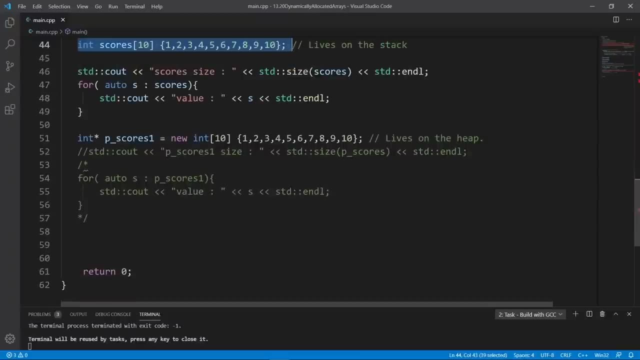 to be cost, like we have with static arrays, and they have a few differences compared to static arrays that were stored on the stack and that std size doesn't work for them and they don't work with range based for loops. other than that, dynamic arrays are really cool and you should use them. 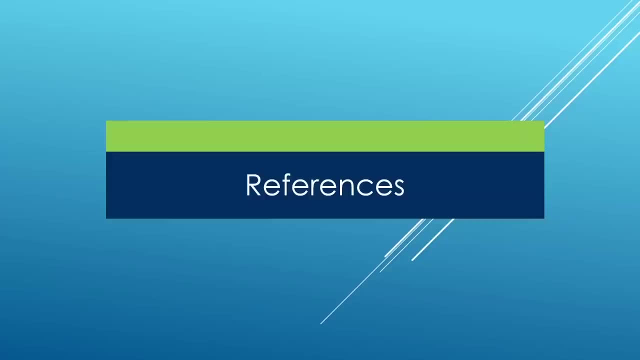 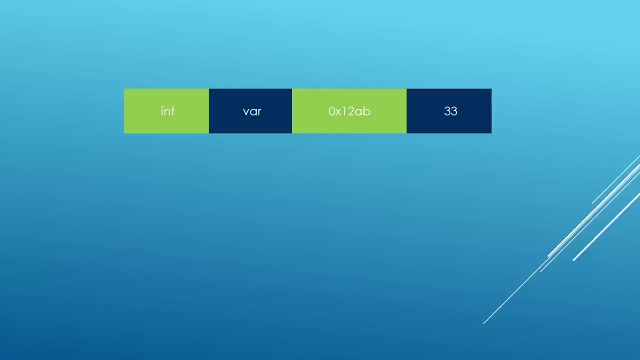 when that helps, whatever it is you are designing. now let's come to this new chapter where we are going to be talking about references. references are a way you can set up aliases for your variables and have other variable names you can go through to modify that same variable. for example, here we have a variable called var. it is an integer. 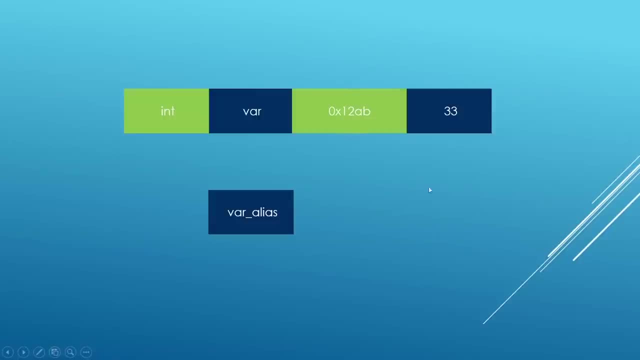 it lives at this address here and the value inside is 33. if we set up another alias to it as var alias variable and use it in pretty much the same way, we use the original variable, and this is going to come in handy in many situations, as we are about to see in this chapter. 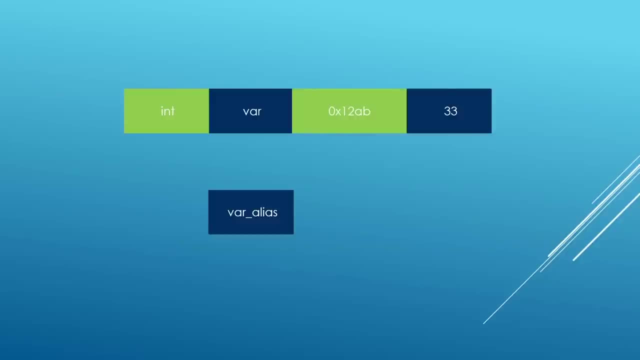 we are going to start in the next lecture and see how we can declare, initialize and use references in our c plus plus applications. go ahead and finish up here and meet me there. in this lecture we're going to see how we can declare and use references in our c plus plus application again. 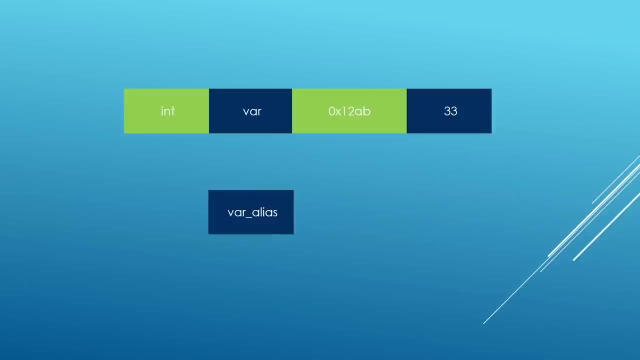 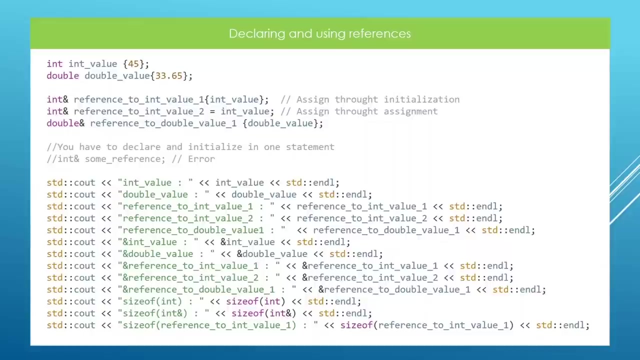 a reference is an alias variable that you can use to reference an original variable and use that reference in pretty much the same way you use the original variable. let's see how that can work in c plus plus. here is a simple example. we have two variables. one is an integer. 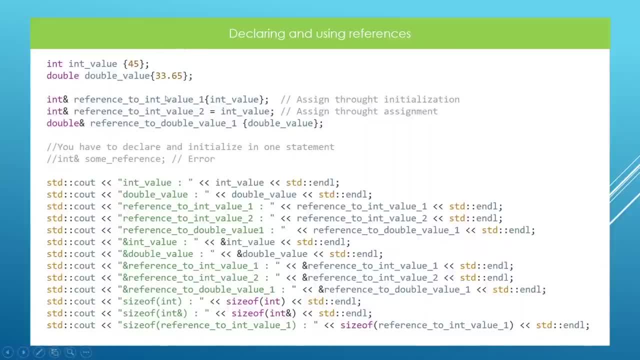 we have 45 and the other is a double. we have 33.65 n. we want to set up references to this variable and the syntax is ridiculously easy for the int value. its reference is going to be something like int ampersand. you put the. 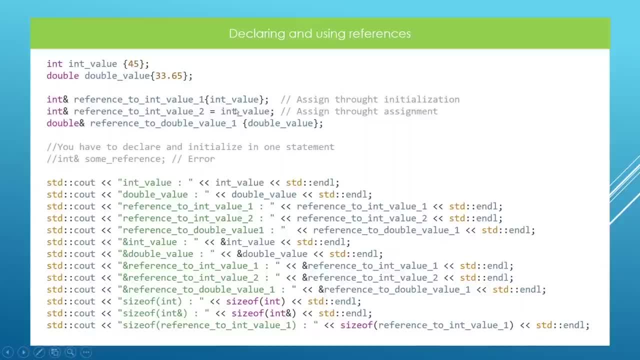 ampersand symbol. you say the name of the reference and you initialize this with the value in the variable that you want this to reference. so reference to int value is going to be referencing our integer here and we can use this name to reference this variable here and it is going to. 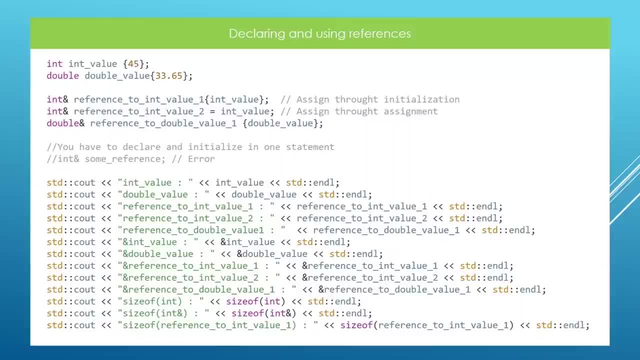 be like. we are using the original variable, which is int value. here you're going to see how this works in a minute. we can do the same using assignment initialization and down here you see that we have an example for the double value and we have a reference to it once we have these. 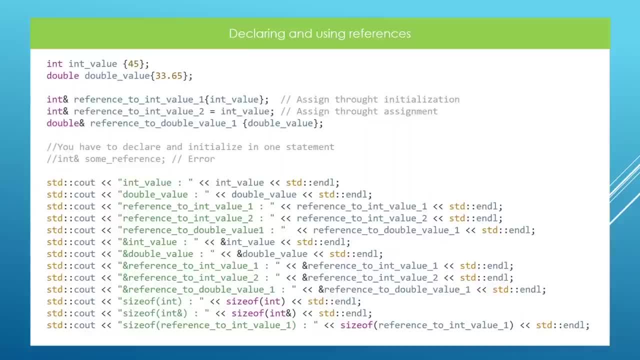 references. we can use them like we use the original variables. for example, if you come here, you see we are printing stuff out. if we print int value, we're going to get the value printed out. if we print double value, we're going to get the value printed out. we can also print through references. you're. 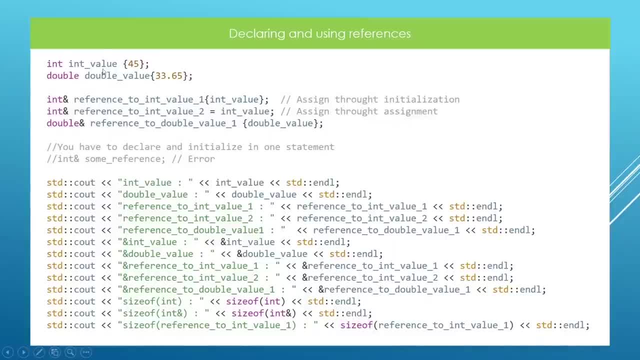 going to see that they are going to print exactly the same value as we have in the original variables. but the interesting thing is going to be that if you print the addresses through the original values and print the addresses through the references, you're going to get the same addresses printed out, which is really going to say these two variable names. 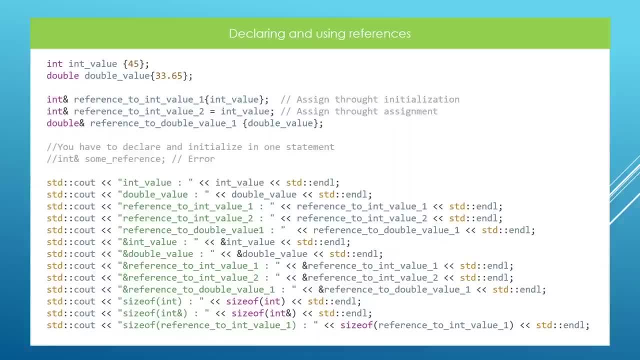 are almost exactly the same thing in c plus plus and this is really cool. you can use the reference as if you are using the original variable name in your c plus plus code, even going to try and go through the sizes and print them out and you're going to see that they. 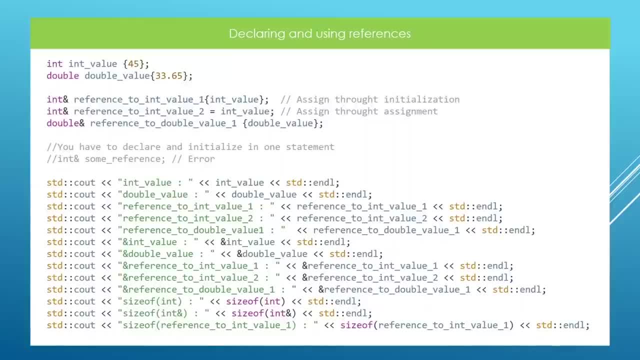 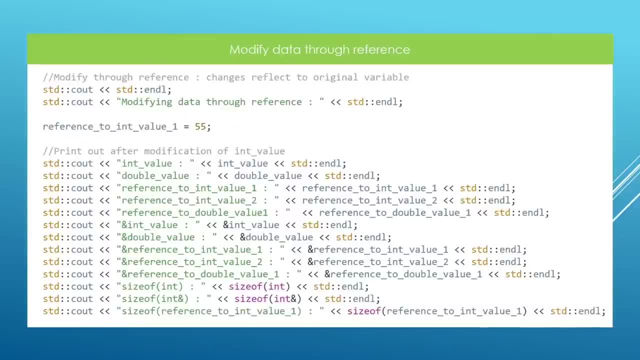 are going to be exactly the same thing and we are going to see how important this can become in c plus plus code as we go through this chapter. okay, now that we have the reference declared, we can go through that and modify the value, and if we do that, the changes are going to be reflected. 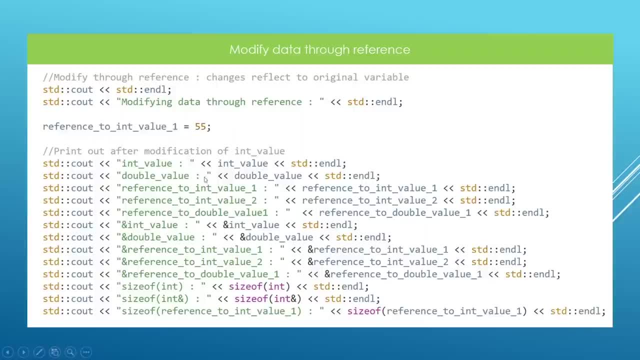 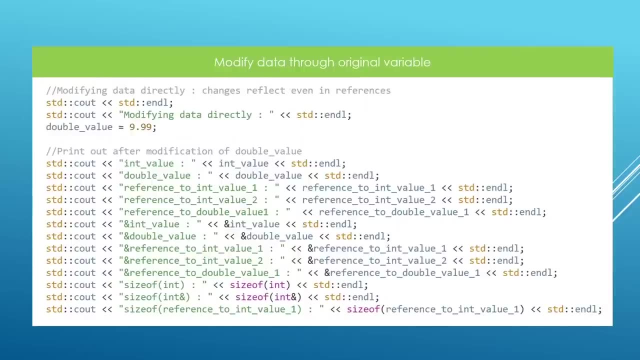 in the original variables and if we print stuff like this again, we're going to see that the changes are going to be reflected in the original variables. okay, if you modify the original variable, the changes are also going to be reflected in our references, and this is exactly what we would expect from our references. okay, so this is. 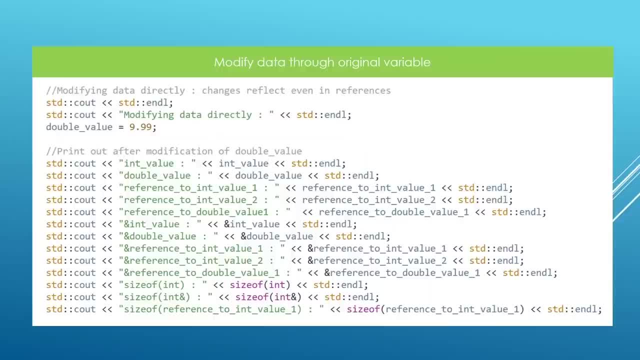 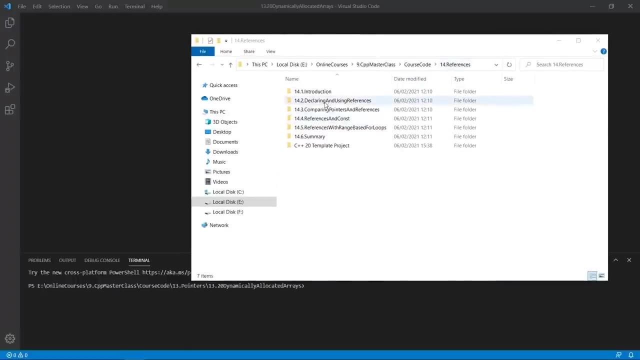 really all there is about references. they are aliases to your variables and you can use them pretty much the same way you use your variables. let's head over to visual studio code and see some of these things in action. here we are in our working directory. the chapter is references, and 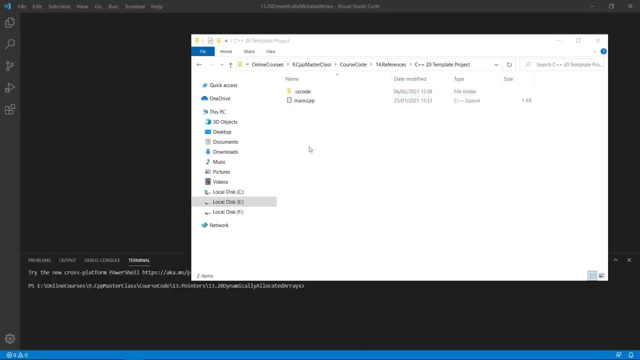 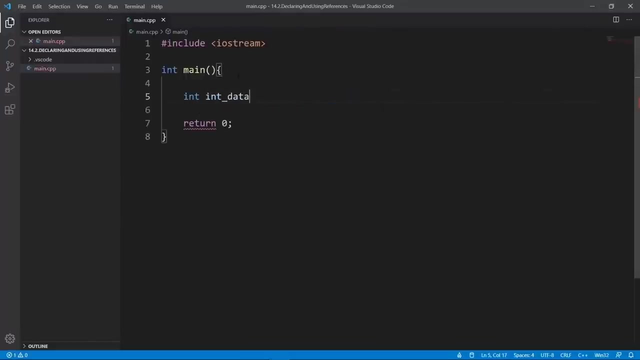 the lecture is declared clearing and using references. we are going to grab our template files here and we're going to put them in place and we are going to open this in visual studio code. we are going to set up an int variable. let's call this data or int data. this is going to be much more. 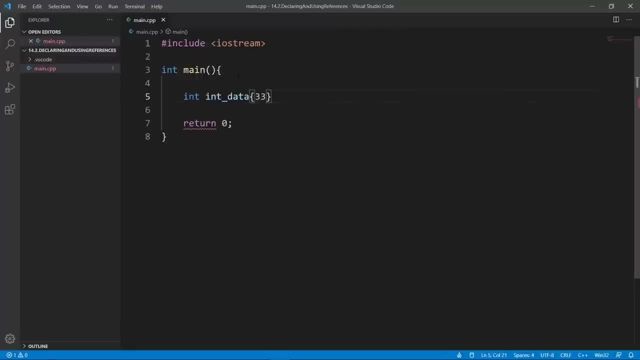 descriptive and we're going to initialize this with a 33- why not? and we're going to do a double and say double data and we're going to put in a 55 in and we're going to set up a reference to these variables. and again, a reference is an alias that you can use in pretty. 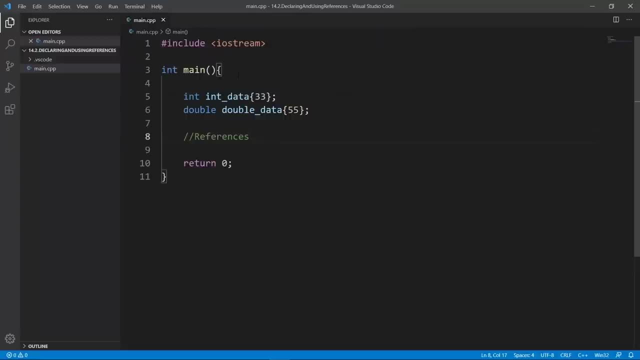 much the same way. you use the original variable. so we're going to set up a reference to int data. we're going to say: and reference mean reference by putting the ampersand symbol here, and we're going to say rough int data and you initialize that with the variable name you want this reference to. 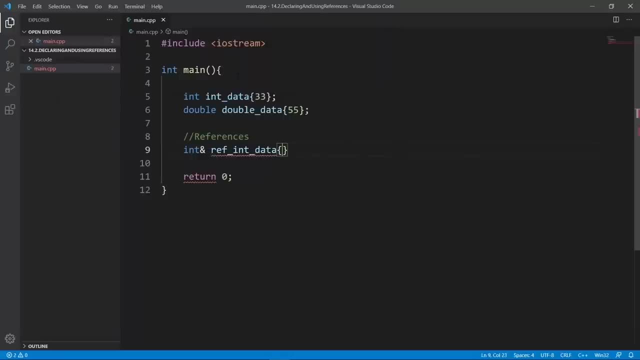 reference. and here we want to reference int data. so we're going to pass in int data and this is going to be it. our reference is declared. we can do the same for double data. so let's do that double and we're going to say it's a reference. we're going to say rough double data and we're going. 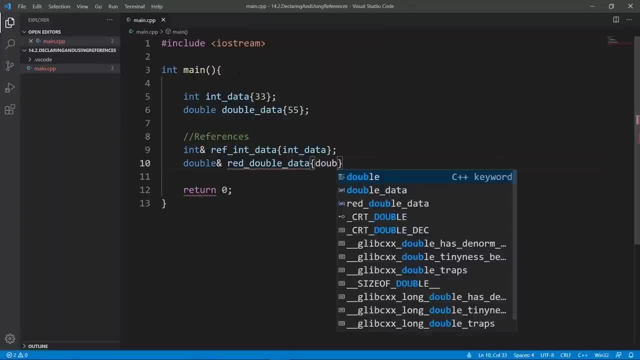 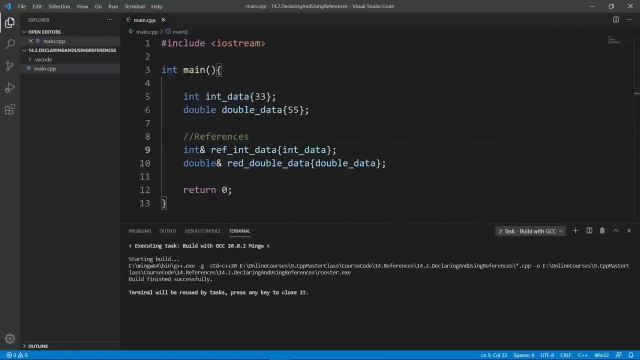 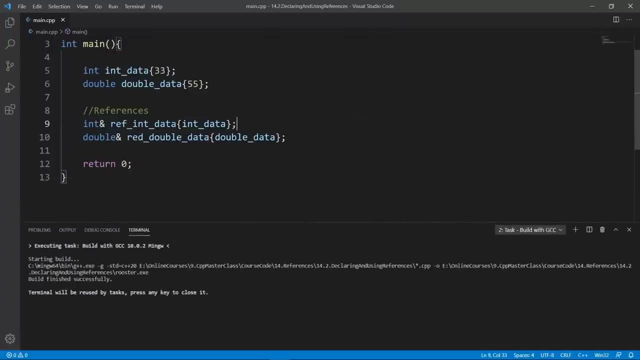 to reference double data here. so let's do that. okay, let's bring up our terminal and see if we can compile this code here. we're going to compile with gcc, like we always do, and let's close this thing on the left because it takes up some of the space here. the world is good, so this syntax is. 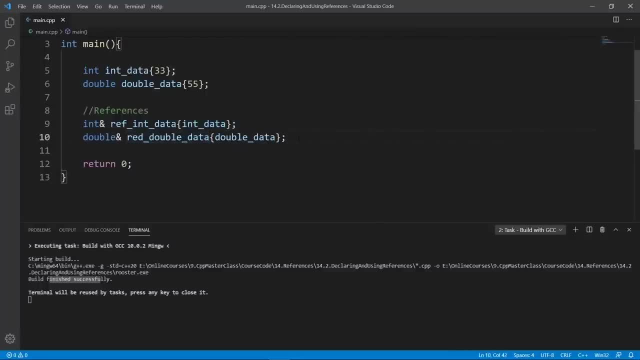 valid c plus plus syntax. so what we can do is read values from all these things and show you that they really are the same things. so we're going to print stuff out and i am going to put here some code and i am going to come back when i have typed this. i don't want you to suffer watching me type these. 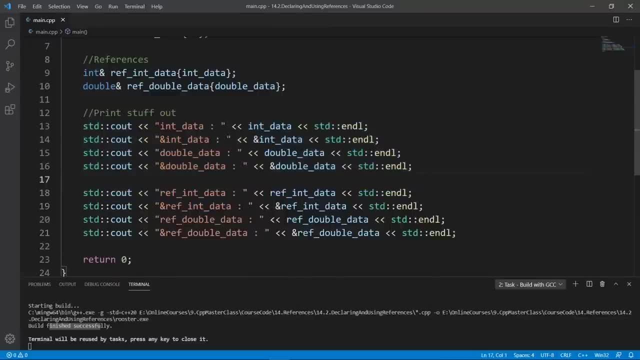 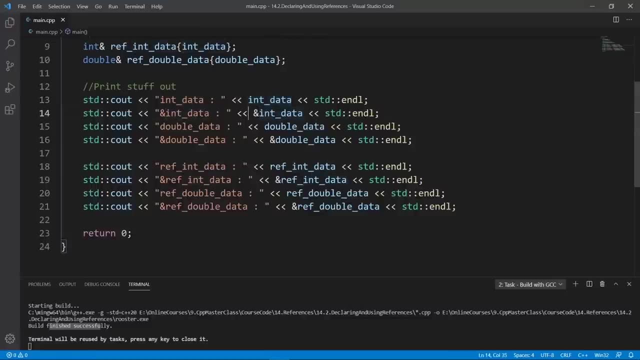 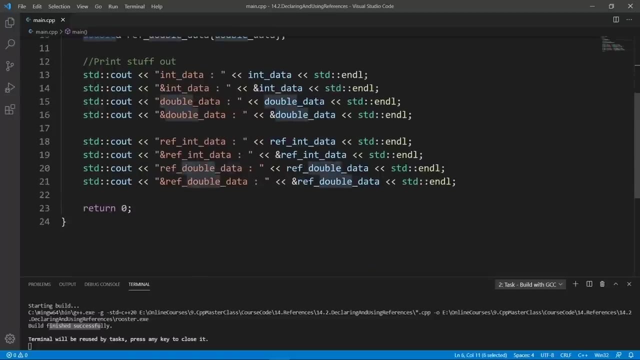 things okay. here i have the code typed down and you see that i am just going to print data through the original variables. i am going to print the actual data and print the address of the variable, and do the same for the double data, which is of type double- how convenient. and we're going to print references. we're going to print the. 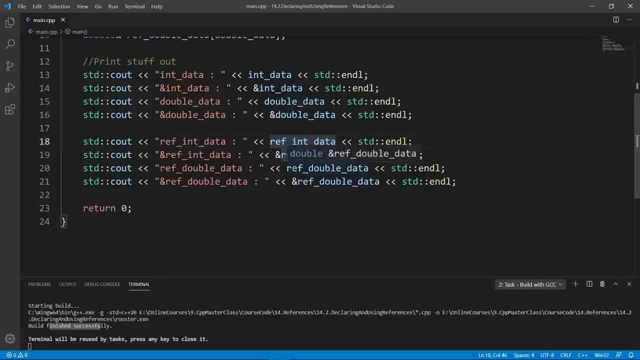 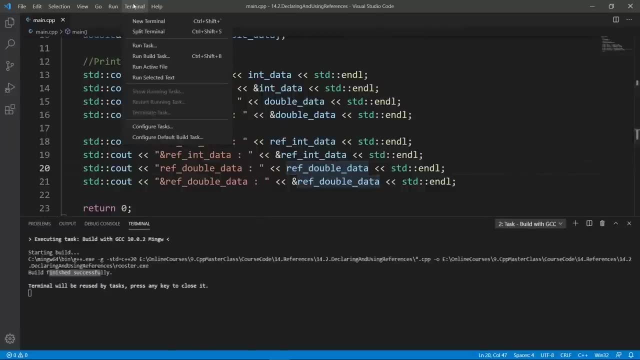 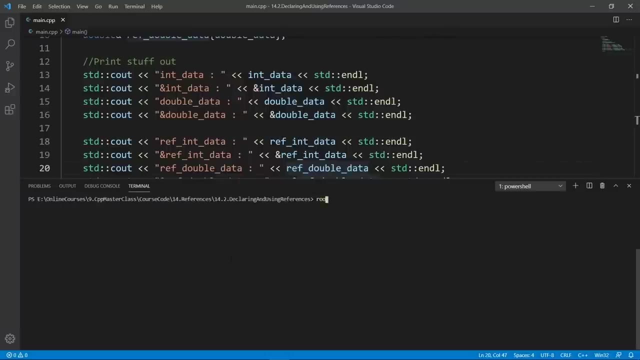 reference and the address of the reference, and we're going to do the same thing for our ref double data here. let's try and world this with gcc. so we're going to run the task to do that and we are going to clear the build is good and run rooster. if we run rooster, you see that, let's. 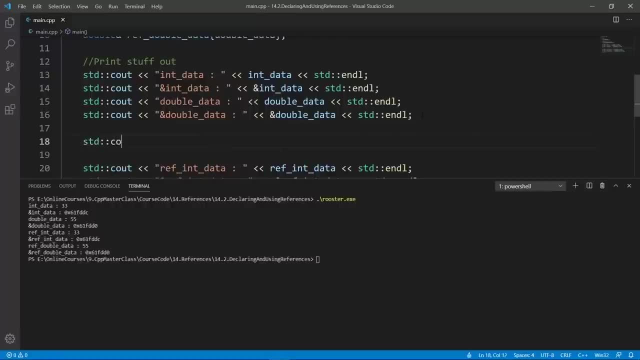 put a secret and the line here so that we see the entire thing. so i'd really like to see my fence easily. so let's do that and build again. okay, the build is good. we can clear and run rooster now and we're going to see the original data enter. data is 33. the address is this guy here we have. 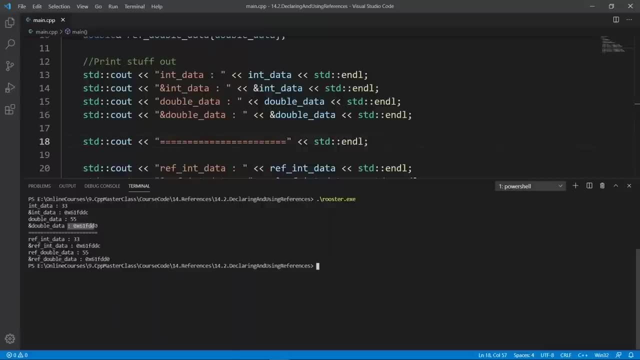 demo data. the value is 55 and this is the Motherboardet info data. the address is 83.3 address. if we look at our references, we have exactly the same thing. the addresses are even the same. it really is like we are using the original variable, and this is really cool. 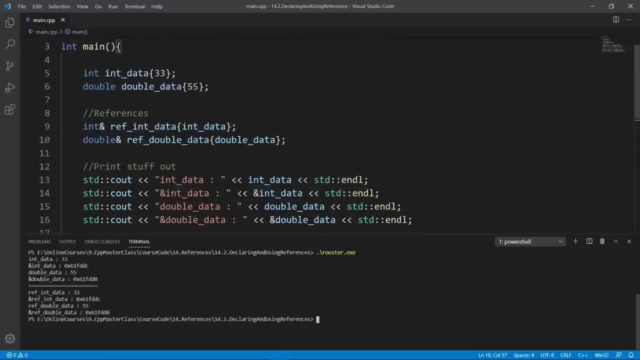 it can allow you to pass data around much easily using references and whatever you are using. when you have sent this data, for example, to some other file or some other function, you're going to be affecting the same data, okay, so you're not going to be making copies and we're going to 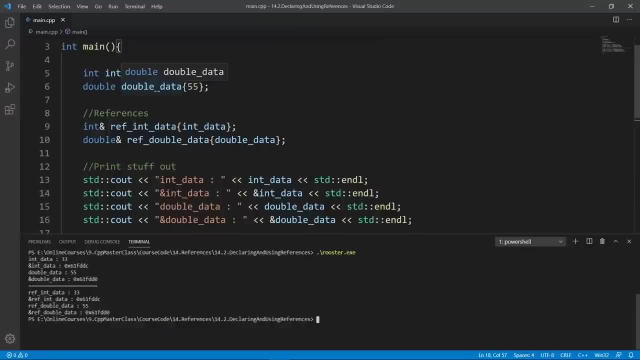 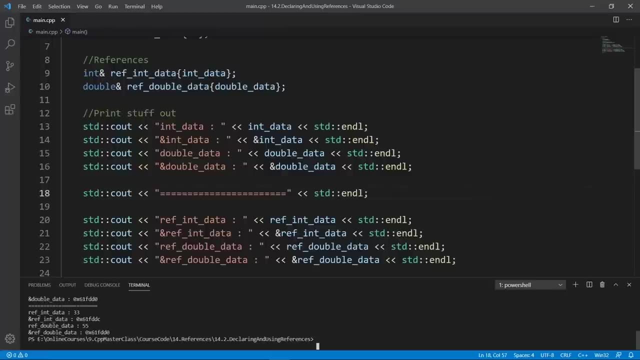 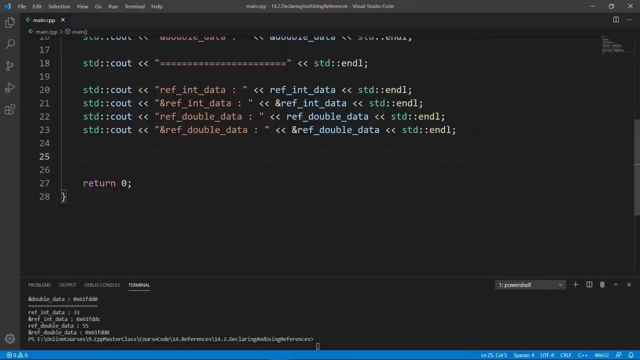 see how cool this can be, especially when we get to working with functions. this is going to be super cool. okay, now we have seen that the references are really referencing the original values. let's try and modify the data through the original values and see that the references are. 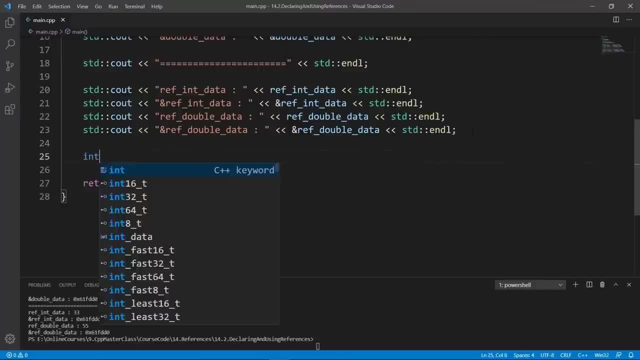 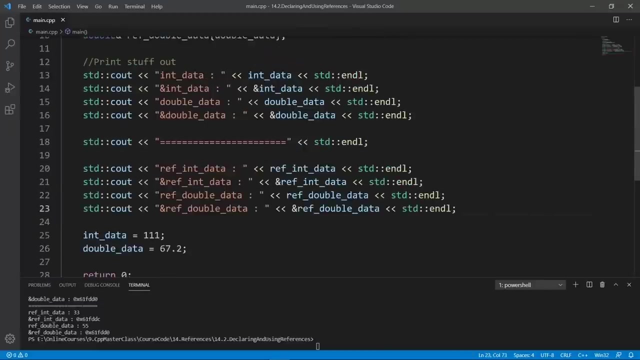 going to pick up the changes. let's do that. we're going to take anti-data and change that to 111, and we're going to take the apple data and change that to 67, point 2.. why not? and after we do this, we're going to print data again, so we're going to grab the. 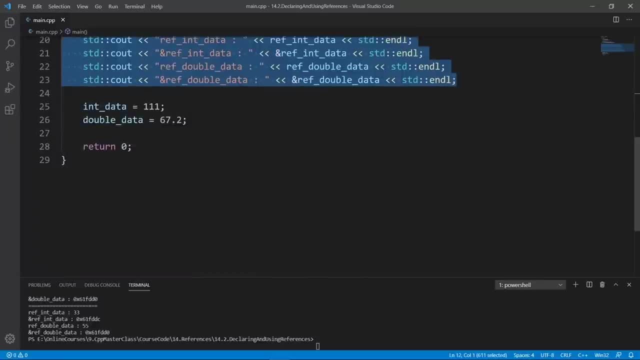 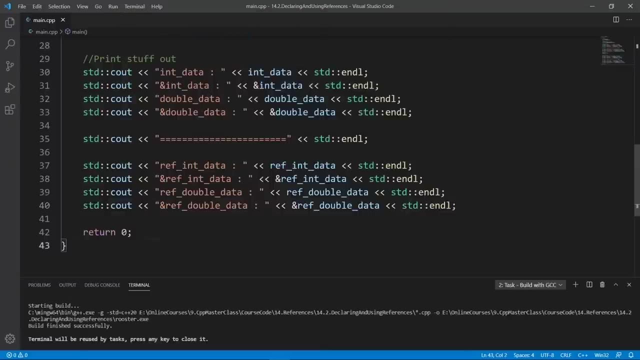 code here and use that again here, and we should see the same changes applied. so we're going to world with gcc, the world is going to be good, as you see here, and if we clear and run rooster, we are going to see that the value is 55. let's put a separation line in here. this is: 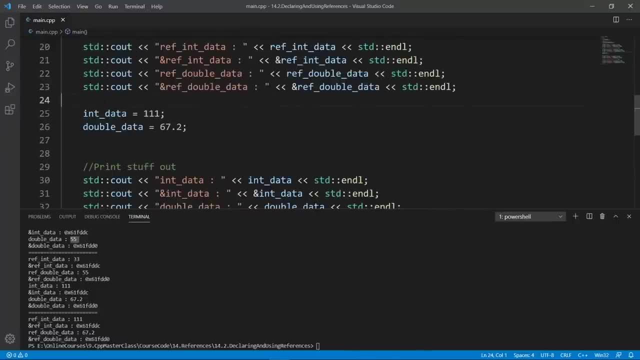 crammed and it is really hard to see what is happening here. so i am going to put an std endl in here and build again. so let's do that and the both is good, so we can clear and run rooster again. and now we see things separated out and it is easier on the eye. here we have int data to b33 and dacodata is 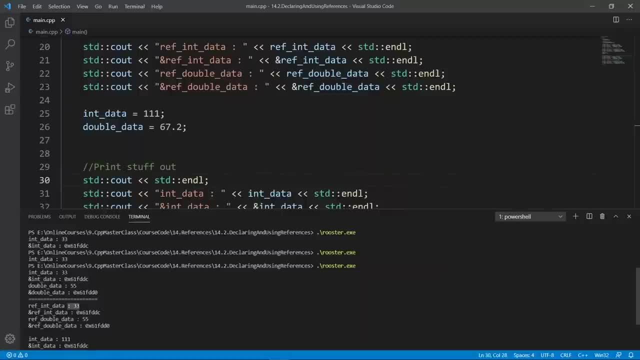 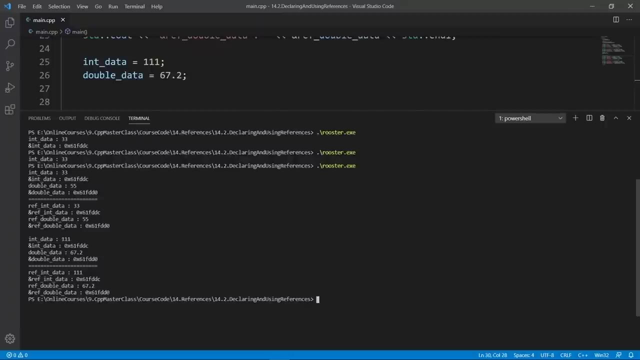 55 and we are going to print our references, which are going to pick up the same things, because a reference is really an alias to the original variables. but if you go down, you're going to see that the data has actually changed: int data has changed to 111 and the double data has changed to 67.2. and the interesting thing- 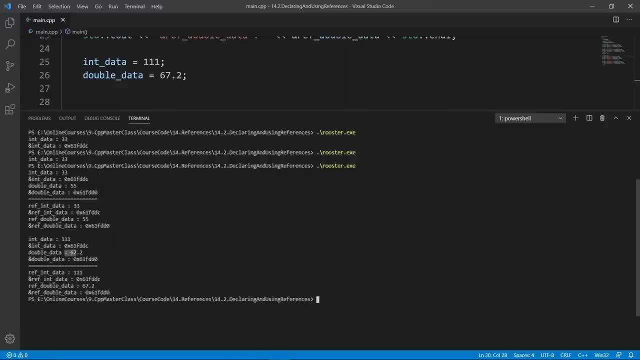 is that the references have also picked up those changes, because they really are referencing the same things in memory. it's like we are using the original variable to read these things, like we are doing with references here, and this is really cool. here we have used the same thing in memory and 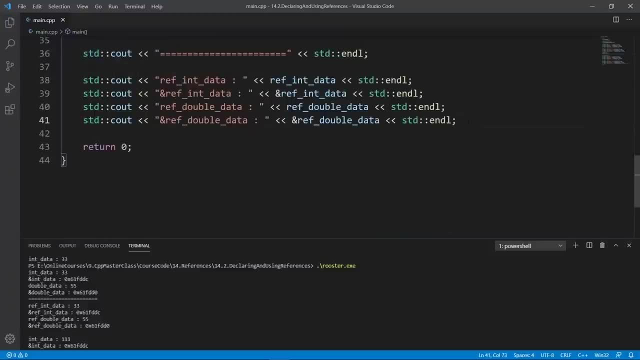 the original variables to modify data. but we can also modify the data through references and the original variables are going to pick up those changes. so let's do that. we're going to say ref int data and we're going to change this to 12, for example, and let's use 1014 or 12.. this is going to 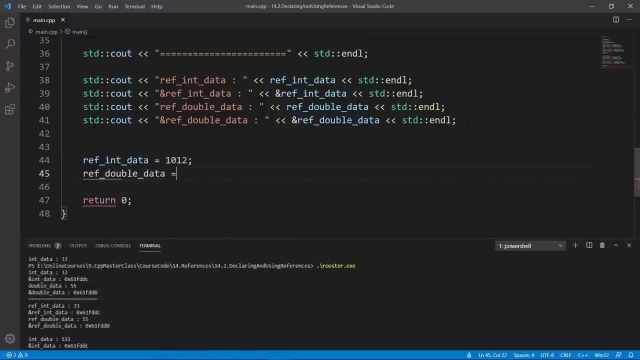 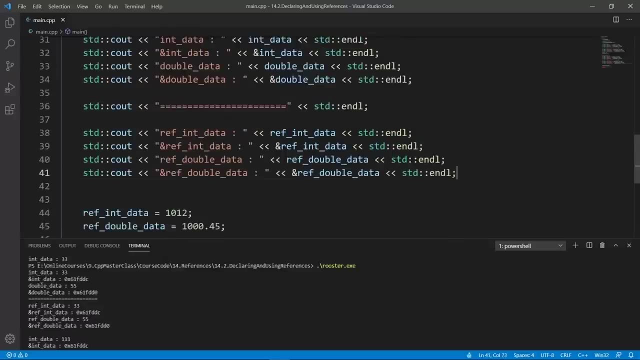 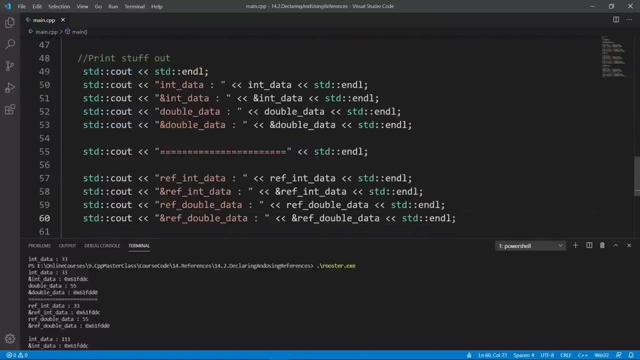 do? we're going to do ref double data and put in another large number- let's say 1000.45, why not? and we're going to print the data again. so we're going to grab this and print stuff out again. so we're going to go down and put in the code to print stuff and you see, it's going to use the. 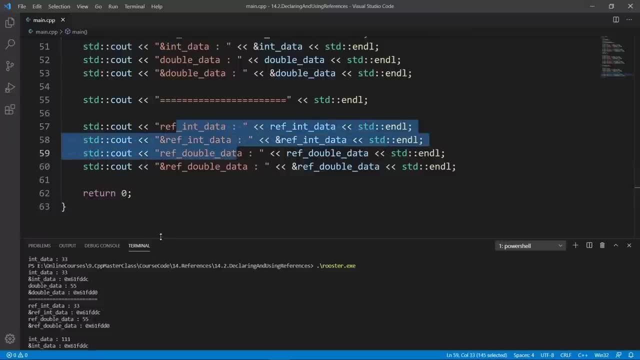 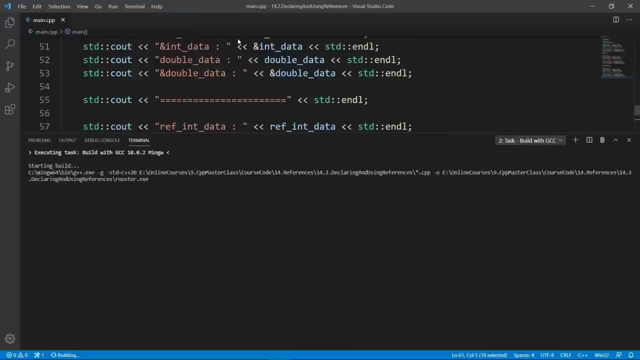 original variables and the references, and we should see the changes reflected in our terminal here. so let's do that and we're going to world with gcc, as we always do. the build is going to be cool. we're going to clear and run rooster. we're going to see that we have 33 and 55. 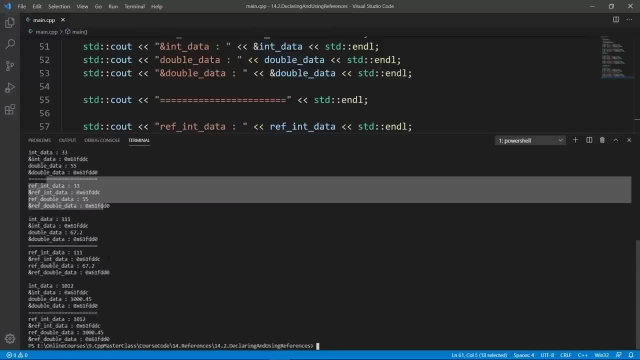 references are going to pick that up. that's what we have here. we're going to put in 111 and 67 through the original variables and the references are going to be picking that up and we're going to use references and modify data. you see that the original variables are also picking that up. 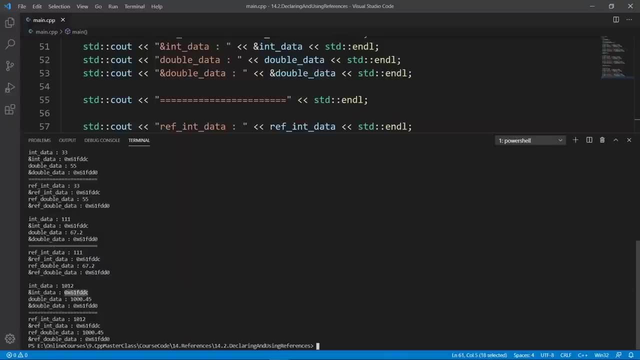 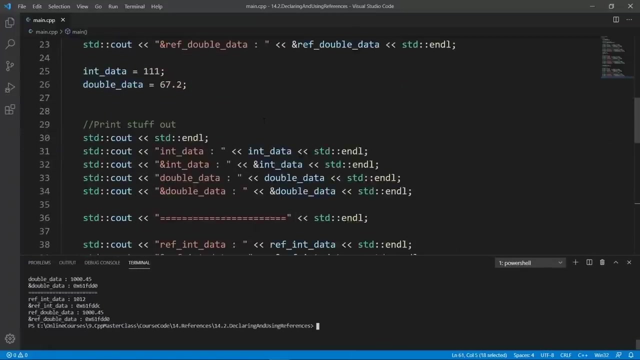 because we are really modifying data in the same memory location. that's why these changes are being shared between references and the original variables, and this is really all we set out to do: how you can set up a reference and prove that the changes we do either through original data- 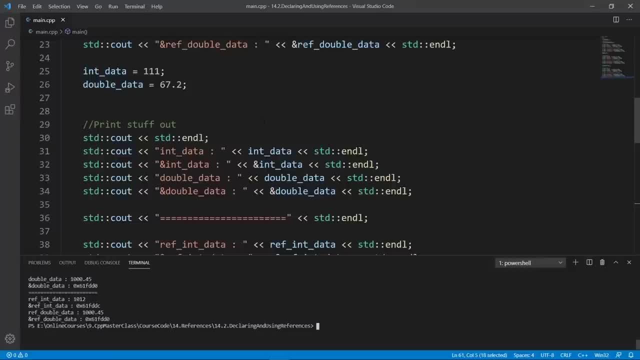 or references are reflected. between these two guys, meaning references and the original variables. we are going to stop here in this lecture. in the next one we're going to do a comparison between pointers and references, because they seem to be doing quite the same thing. go ahead and finish up here and meet me there. in this lecture we're going to be looking at the 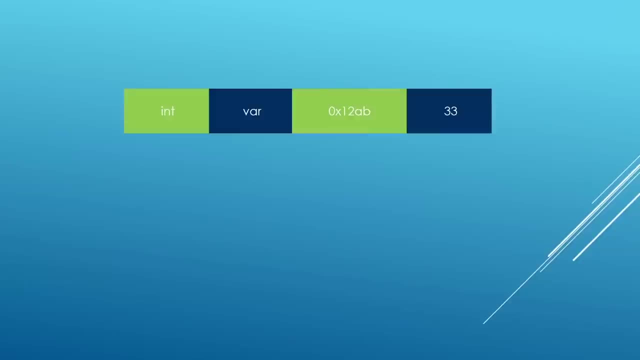 differences between references and pointers. okay, we know that a pointer is really something that is going to store the address of the variable and we can go through that pointer and modify the original variable or really do things with that. but in the last lecture we saw that we could. 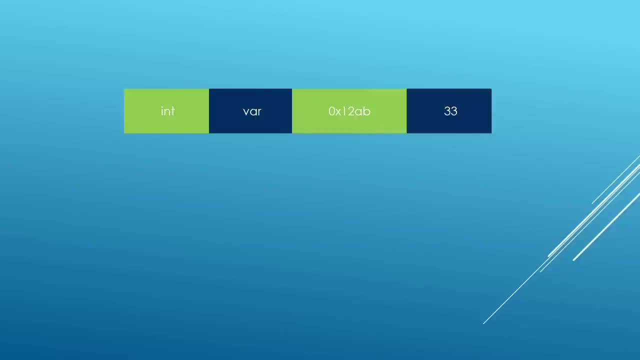 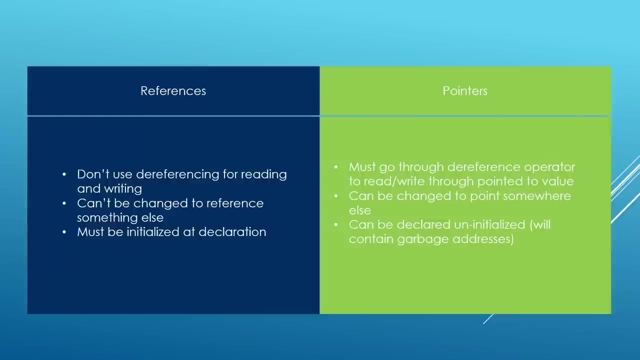 also do the same thing with references. so why have these two mechanisms in place and what are the differences between them? here is a simple slide that i put together to put the important points about references and pointers together. the first thing is that if you use references, you are not going to go through the star symbol to the reference and get to the value you are. 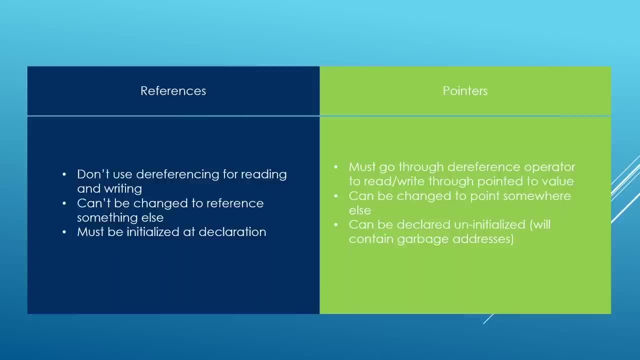 manipulating. so that's going to really feel like you are using the original variable, but with pointers you are going to go through the referencing. so that's the first difference. another thing about references is that you can't change them to reference something else later. but with pointers we saw that we could do that. we can. 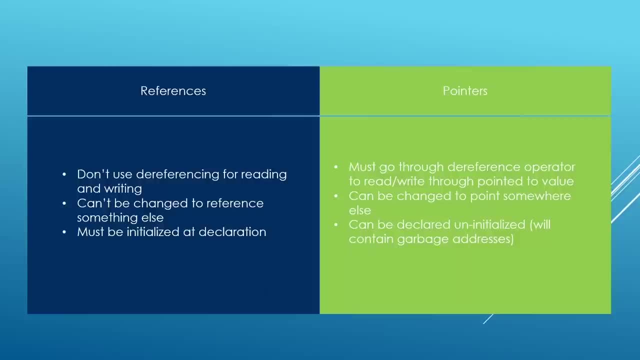 change a pointer to point somewhere else if it happens to be a non-const pointer. the other thing is that for references you have to initialize them at declaration. you can't declare a reference and not initialize that. if you do that you're going to get a compiler error and we're going to see that. 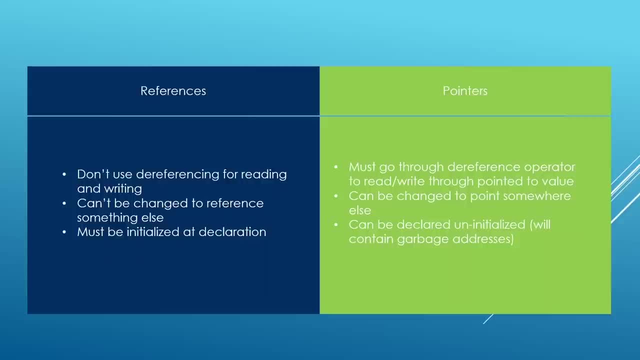 in a minute. but for pointers, you can declare a pointer and not initialize it and it is going to just contain a junk address. and if you try to use that uninitialized, you are going to be setting yourself up with a pointer and not initializing it. and if you try to use that uninitialized, you are going to be setting yourself up. 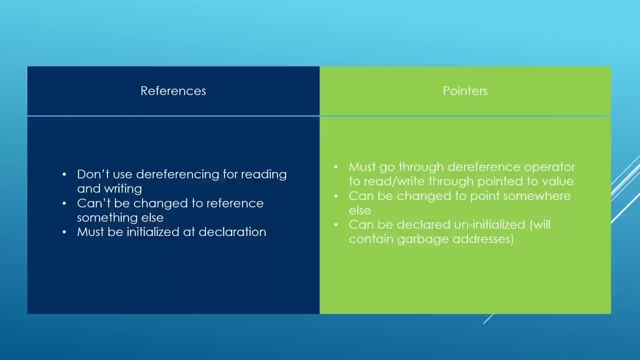 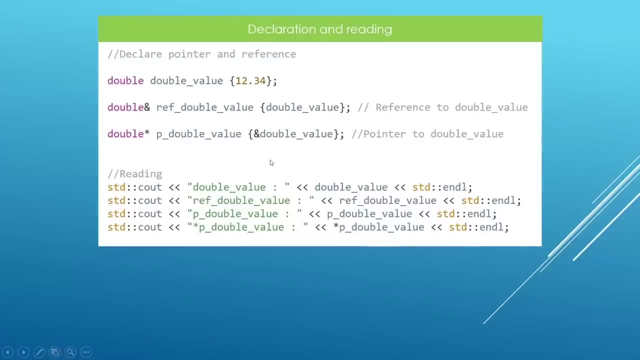 for trouble. so we saw that. so these are the main differences between pointers and references, and now we are just going to be looking at how these translate in code. here is a simple example. we have a variable called double value, which happens to be double, and we have a reference to it and a 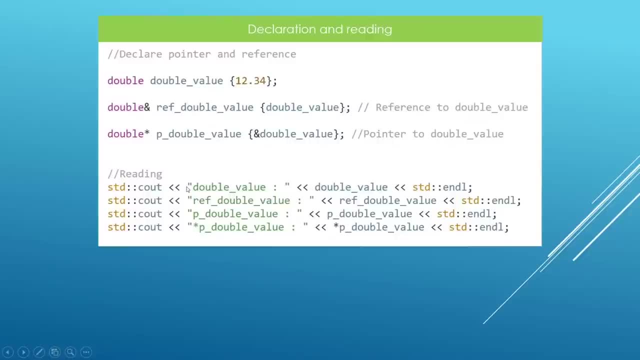 pointer to it. so you already know these concepts. now, if we want to read the value in here through our pointer and references, we're going to be using two different syntaxes. if we go through the reference, we can use this reference variable name directly and read the value or change it. 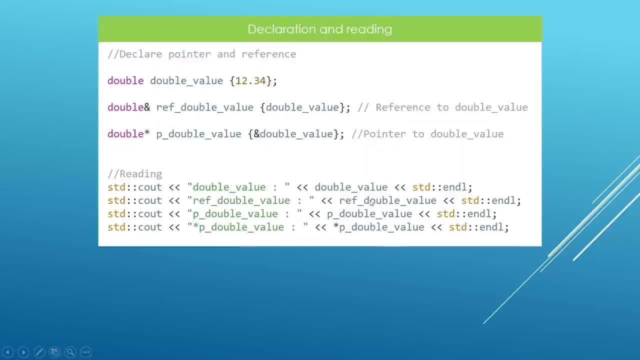 and we can do something like ref double value to print that out. this is going to work. but if we want to go through the pointer we will have to go through the referencing, and this is really bad. you know, sometimes people don't like this syntax. they think that it is not direct enough, so they 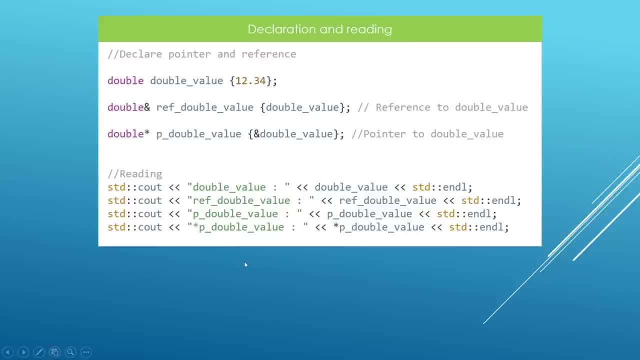 prefer to use references to do these kinds of things. but pointers are still important, as we will see later as we progress in the course. so this is one difference. with references you don't have to go through the dereferencing mechanism to use this star here to print stuff. 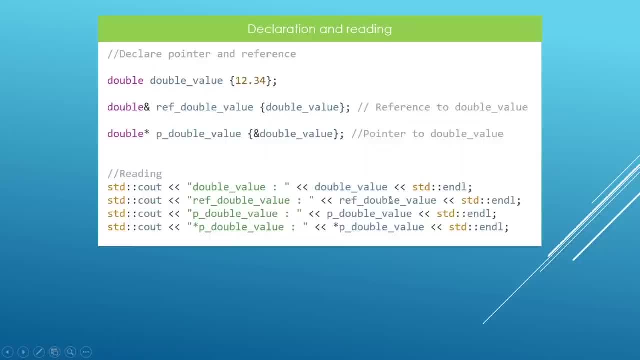 or even manipulate the data inside. you just use the variable name and it is going to work with pointers you have to reference, because if you don't the reference you're going to be referring to the address stored in this pointer. this is the first difference and we see that the same applies. 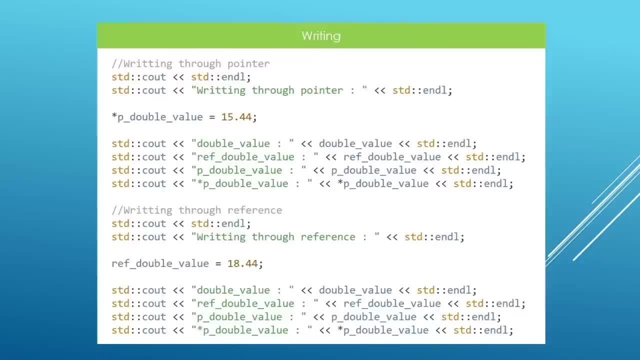 if we are trying to write data into our variable. if we go through the pointer, we will have to dereference and use the star symbol in front here. if we are using a reference, we can do that directly, as if we are modifying the original variable. so this syntax is much more readable. the other difference is that we 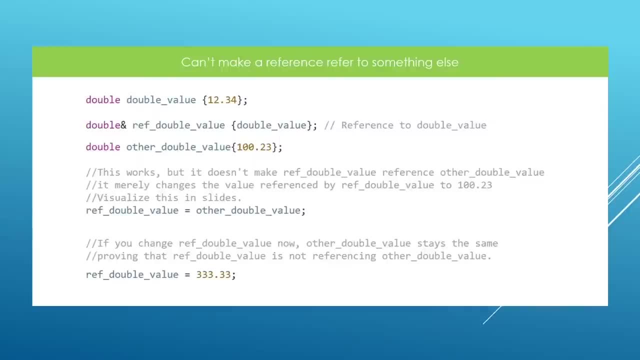 can't make a reference reference something else, but we can change a pointer to point to something else. let's look at an example. here we have ref double value, which is a reference to double value, and here we are doing an assignment to this thing. here we are saying either double value and 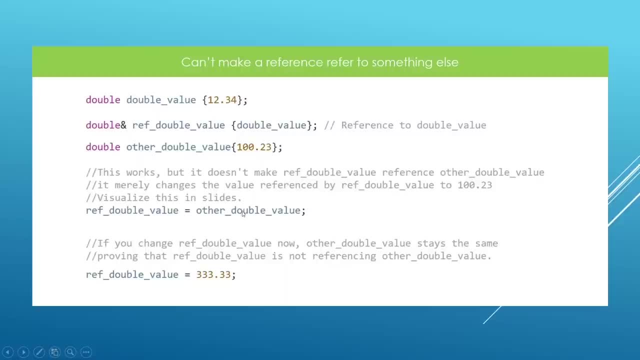 assigning that to our reference. but what we are doing here is not making ref double value reference this other variable. we are just grabbing the value in other double value and assigning that to our reference and the value in other double value is going to be reflected in the original. 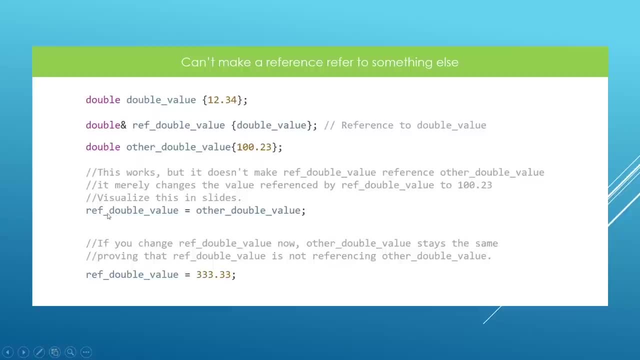 value here. so this is what we are doing. we are not reassigning to our reference to make it reference something else. we are assigning the value to the reference as it is now and it is going to be still referencing the same variable in memory. if you print out the address in memory, you're going to see that the address of the reference here. 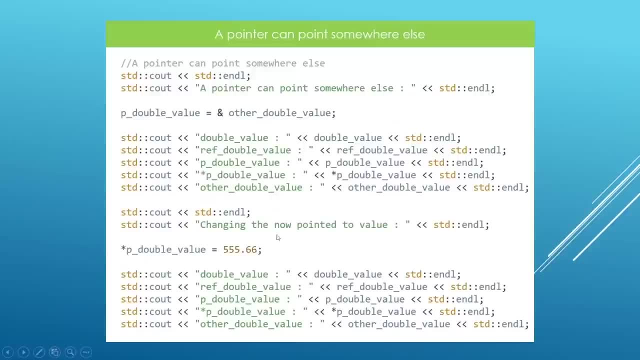 hasn't changed. so this is something you should keep in mind. but we know that a pointer can point somewhere else. if we have a pointer here, for example p double value, we can reassign it another address and make it point to that new address. so in this regard we 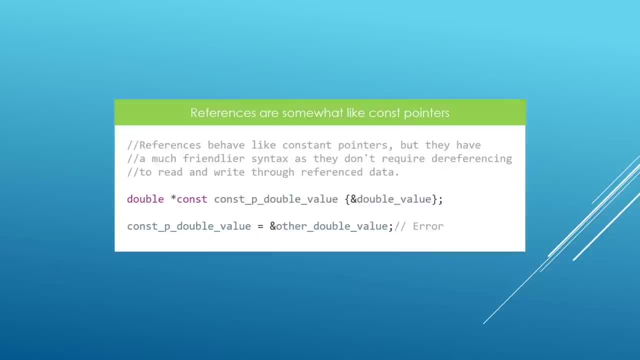 can think of references as const pointers, because const pointers can't also be made to point somewhere else. and if you're trying to do that, for example, here we have a cost pointer, it is called const p, double value, and if we try and make it point somewhere else through, 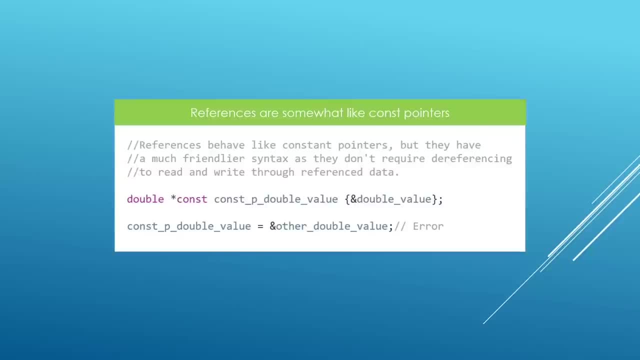 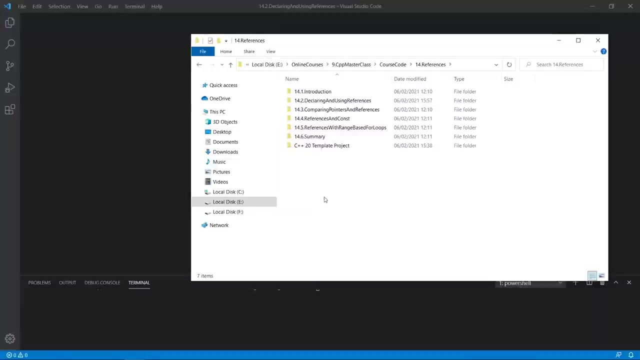 this assignment. here we're going to get a compiler error, okay. so this is really all in terms of the reference that we had to make between references and pointers. now we're going to head over to visuostudio code and see how these things work in real code. so here we are in our working folder. 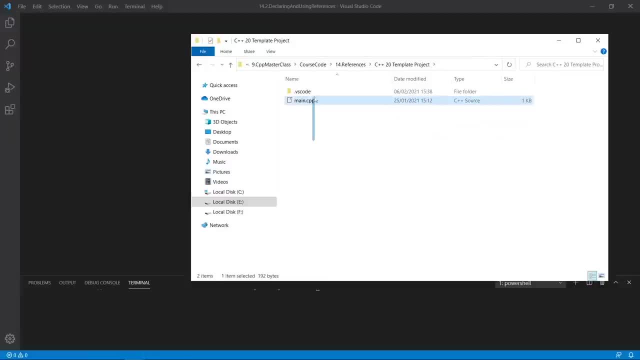 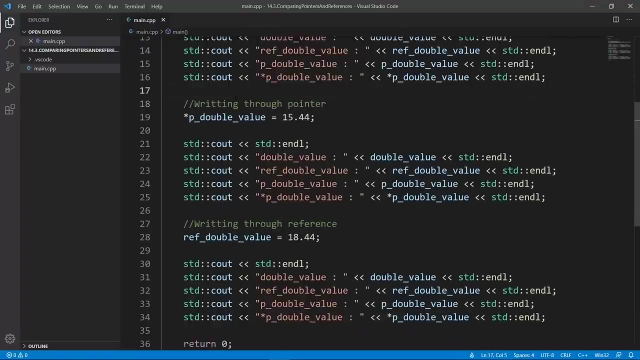 the current project is comparing pointers and references. we are going to grab our template files and put them in place and we are going to open this project in visuostudio code, like we always do. we are going to go down and put in some starter code and let's align this a little better. 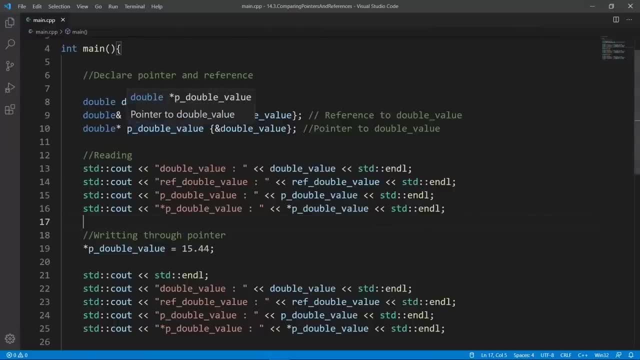 so and we can close this pane so that we have some breathing room. here. we have a variable of double type and we set up a reference to it and a pointer to it. this is how we do this. thanks, you already know this, and we can try and read through the original. 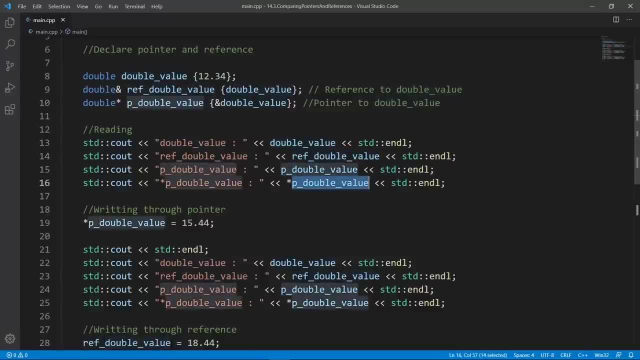 variable through the reference and through the pointer and see how these syntaxes differ and how one might be better than the other. for example, if we look at how we are using the reference, it's really like we are using the original value here. we don't have to do reference if we try to print. 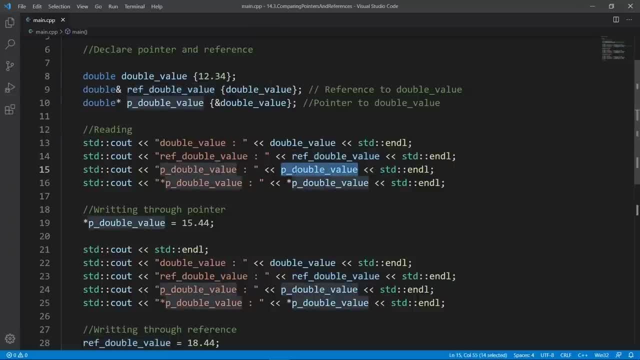 the pointer directly, like this, without the reference end. this is going to print the actual address stored in this pointer. it's not going to print the actual value stored in the address pointed to by this pointer. i really want this to be clear. so this is the syntax we can use. 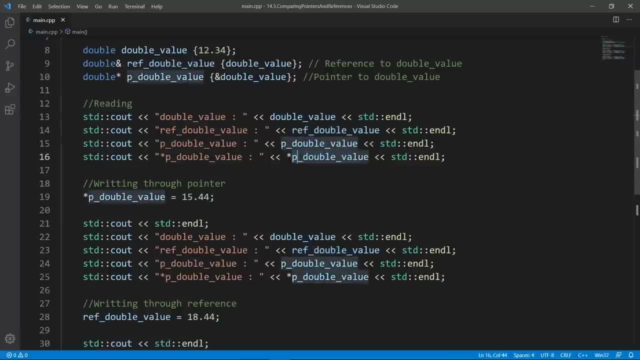 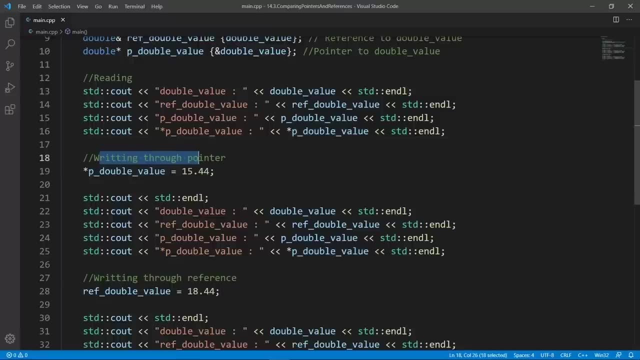 for reading stuff, either through references or pointers. we can also use these syntaxes to write stuff into our variables. for example, here we can go through the pointer and we have to the reference and we can go through the reference to really do the same thing. and we're going to see that. 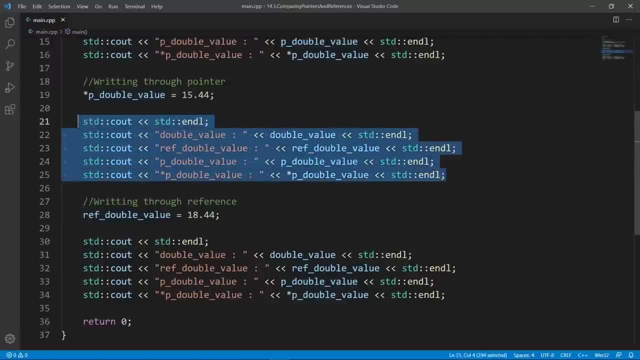 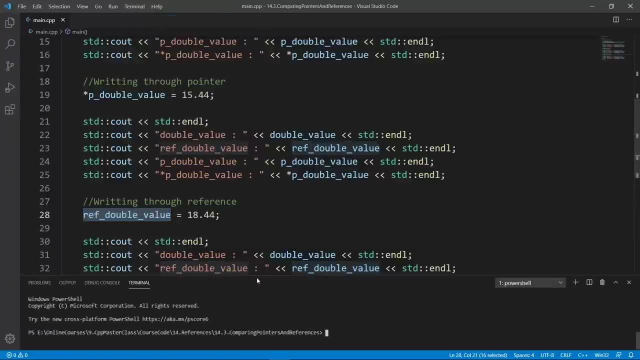 our syntaxes here are going to pick up the changes, regardless of whether we write through pointer or a reference, because all these things really are going to be referencing the same location in memory. let's try and bring up a terminal here and we are going to weld with gcc. let's do that. 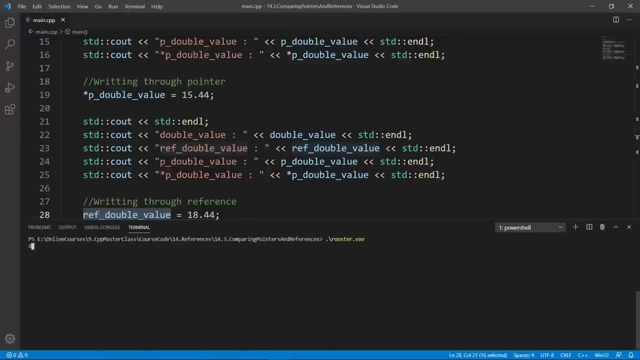 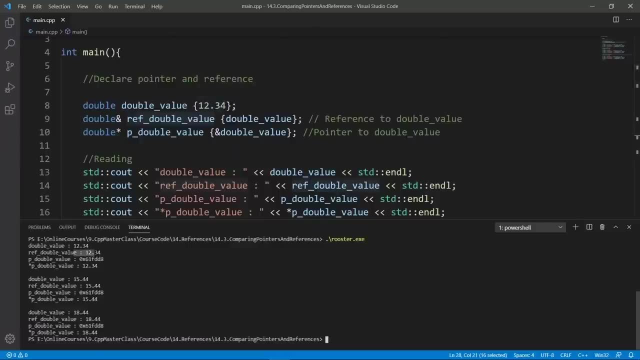 the book is going to be good and we're going to clear and run roaster and you're going to see that at first we're going to have a 12.34 in. that's going to be the value. we can get it through original value, the reference or the pointer, through the referencing and the address is this: 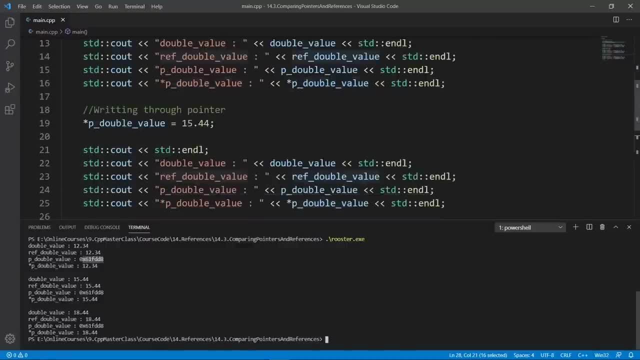 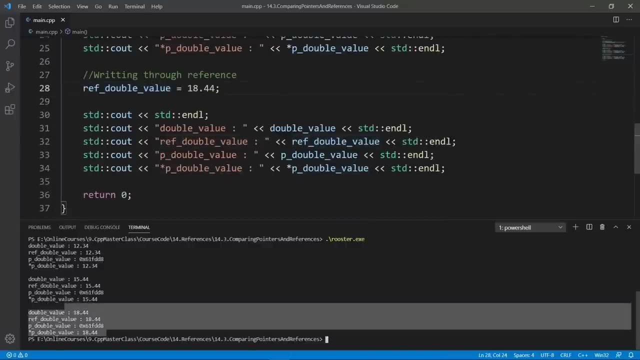 one here: if we change the value through the pointer, we're going to see that the address is going to see the changes reflected here, and if we change the value through the reference, we're going to see the changes reflected in here. so this is how you can use pointers and references to do. 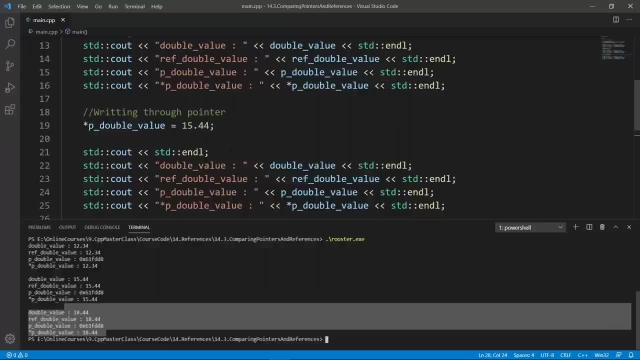 these things here and you can really choose what makes sense for your application. they mostly do the same things, but some people say that the syntax to dereference the pointer here is really ugly. that's why most people prefer to use references like this, but references have other. 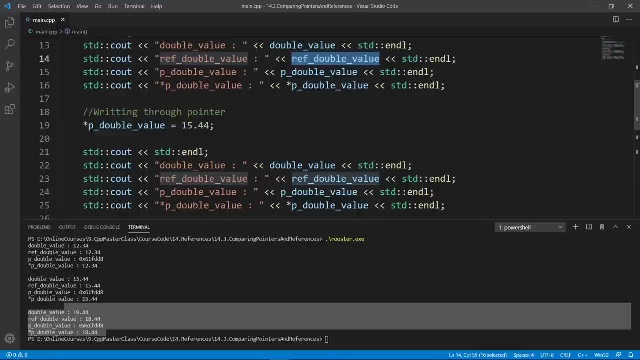 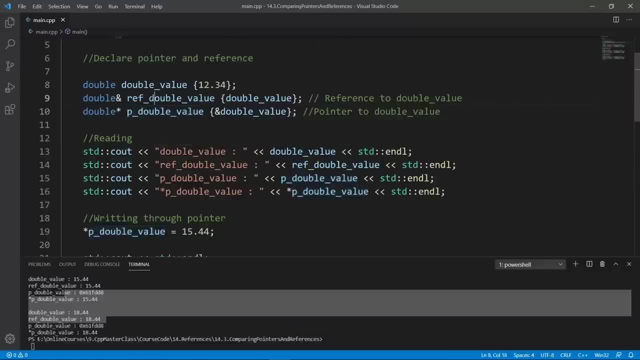 benefits as well, as we're going to see as we progress in the course. another thing i want you to see is that you can change a reference to reference something else in memory. for example, here we have our reference which is ref- double value if we try and make it reference something. 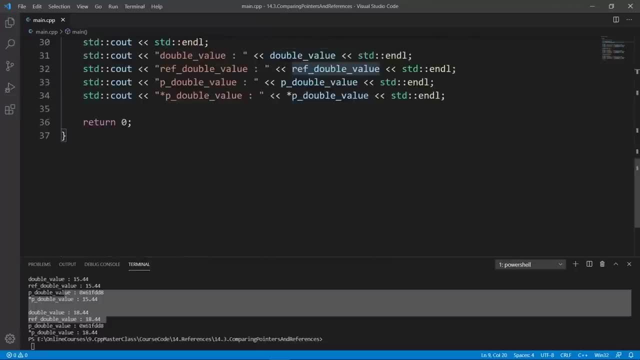 else we're not going to get that result. let's go down and try to do that. so we're going to set up another double variable. so if we try to make our ref double value reference this guy, the syntax that comes to mind is saying ref double value and assign that the some other double value. 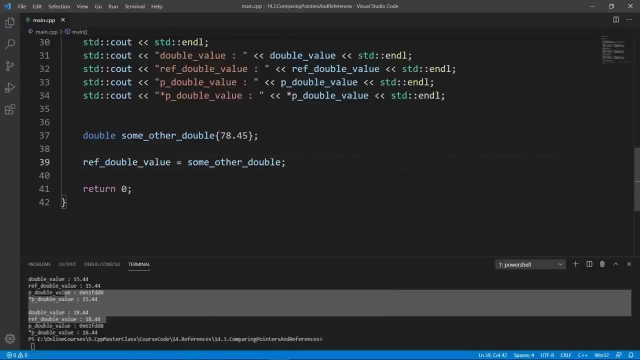 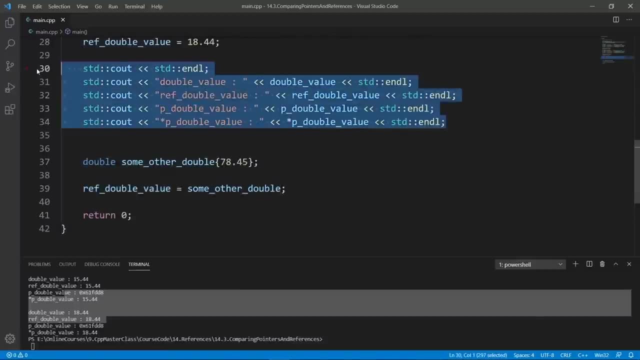 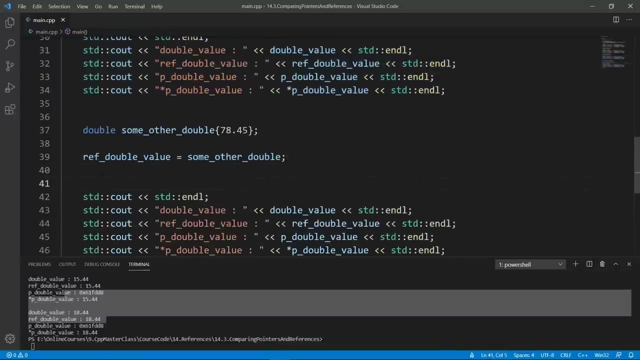 here. now let's see what happens if we do that. we're going to try and print whatever we have in memory using the ref double value here. let's grab this and go down here and say that we are changing the reference, making the reference reference something else. let's say that. so if 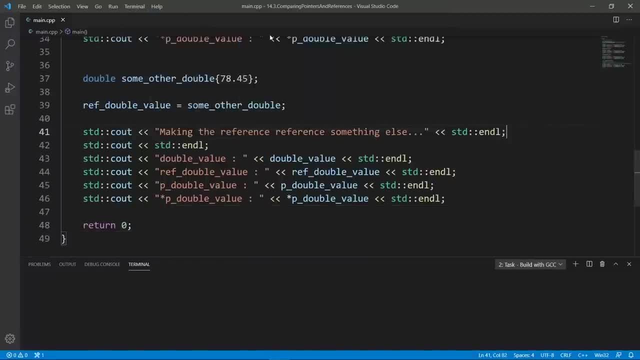 we try to bulk this. let's see what we get. we're going to run and build with gcc and we're going to try and run this clear, not clear, and we're going to run rooster. we're going to see that the last line of output. 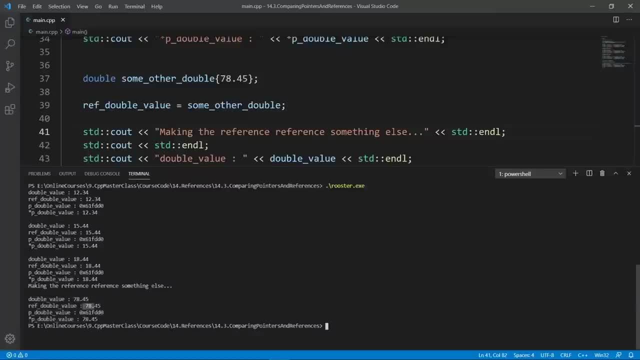 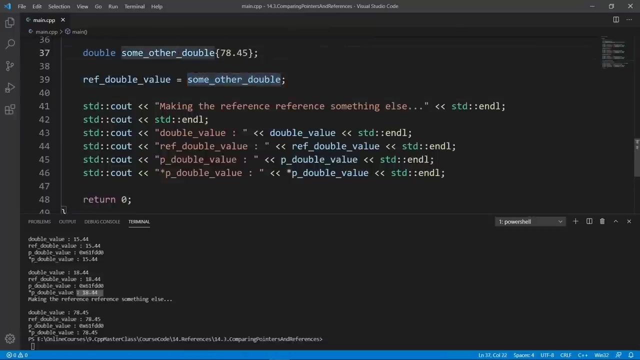 here say 78.45, but the address is still the same. so we are still referencing the same memory with our reference and what we just did here was just grab the value in some other double value and assign that in here. but the reference is referencing the same memory. 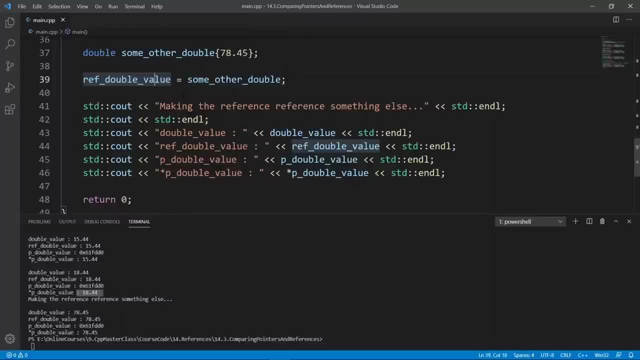 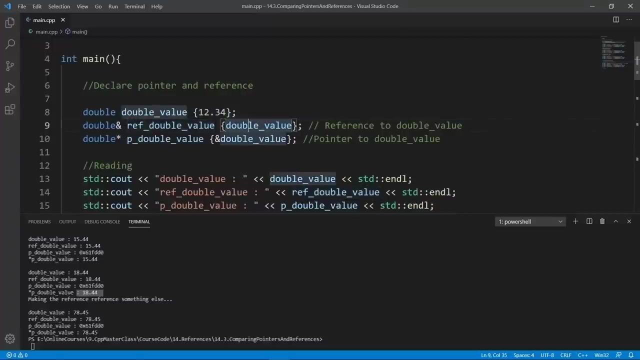 location it's been referencing. so in c plus plus, you don't have a way you can go through to make a reference reference something else. the only chance you have to make it reference something is through declaration here, and that's the reason you can't declare a reference and not initialize. 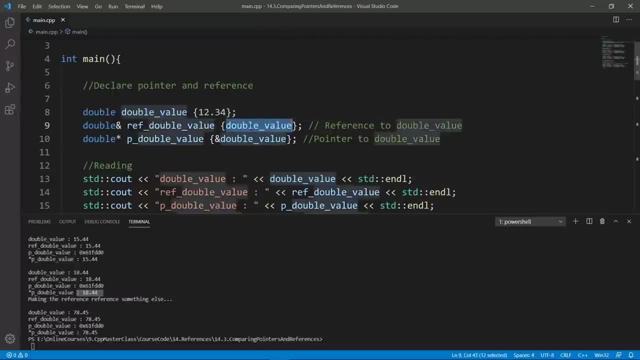 it. if you do that, you're going to get a compiler error, so let's go ahead and do that. and we're going to define a reference with a reference, so let's try and do something like this: we're going to take out this double value and the moment we do this, you're going to see that Visual Studio code is. 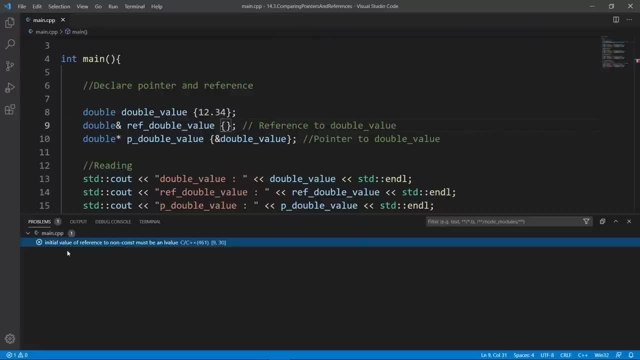 going to be unhappy. you see the squiggly line and it is going to say initial value of reference to non-costs must be a nail value. so what is that? okay, if we take out the initialization altogether, it's going to give us a better error. i think reference variable requires an initializer. 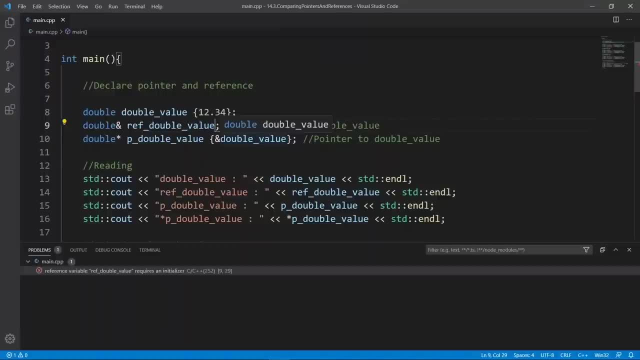 so every time you declare a reference, you have to initialize it, And we should do like we just did before here And we're going to be fine Again. you can't declare a reference and not initialize it. If you do that, you're going to get a compiler error. 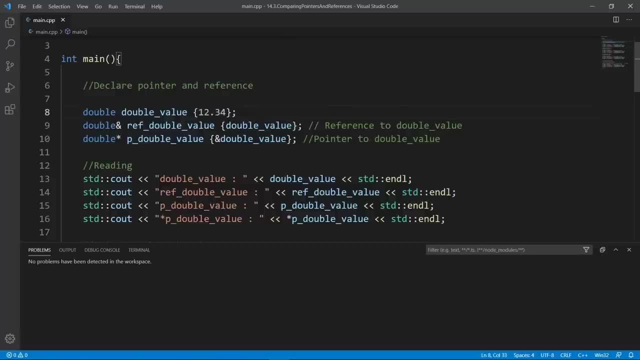 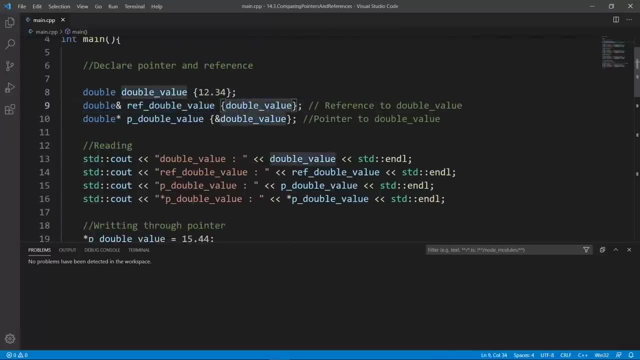 And the reason is that this is the only shot you get to make your reference reference something else. okay, If there was a way for you to bypass this and let the compiler compile this, you would never get another chance to make this guy actually reference something. 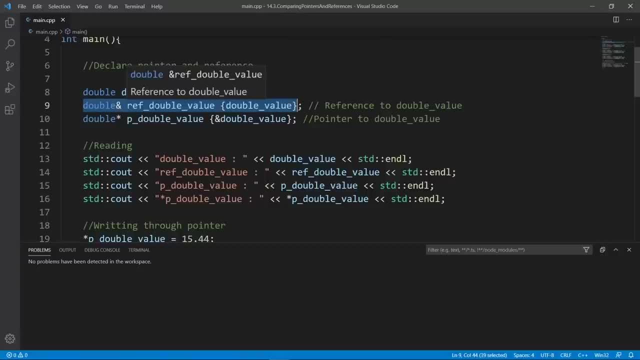 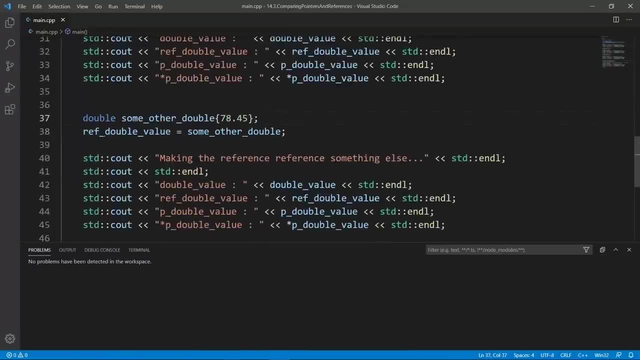 And it would really be a useless reference. So make sure you understand this: You can't make a reference reference something else And if you're trying to do something through a syntax like this, you're going to be assigning the value of whatever variable you have to the reference. 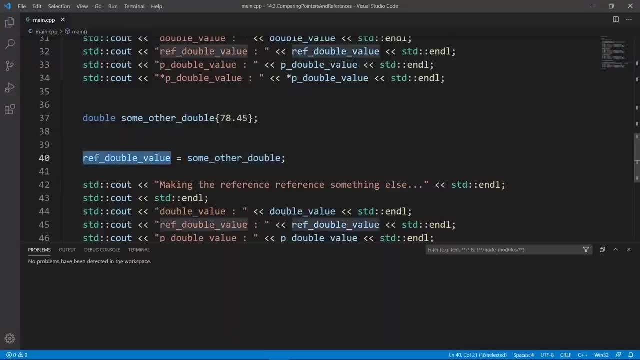 You're not going to be making the reference referencing something else. The reference is going to keep referencing the same variable in memory, as we have seen here. So let's say what we were trying to do here, But we know that we can make pointers reference something else. 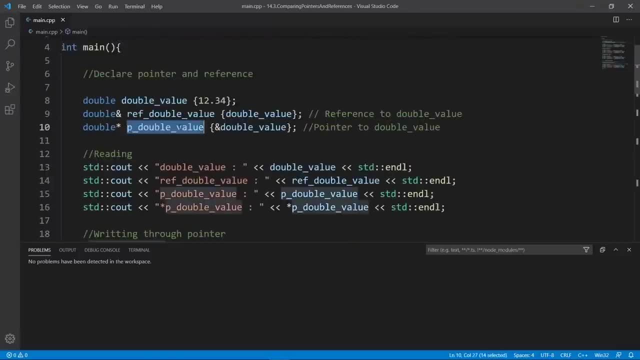 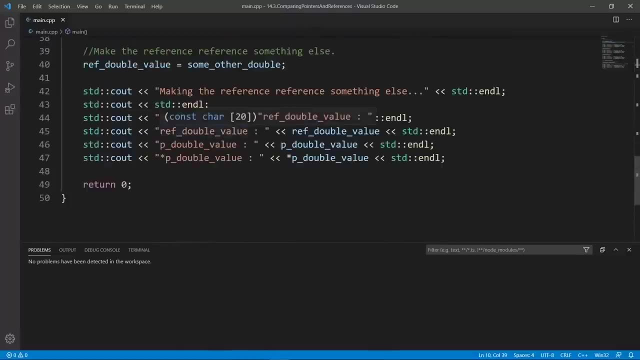 So here we have a pointer again, this pointer called the pdouble value and it has the address of double value inside, but we can set up another variable okay, So we can make that reference, this other variable here, And let's do that. 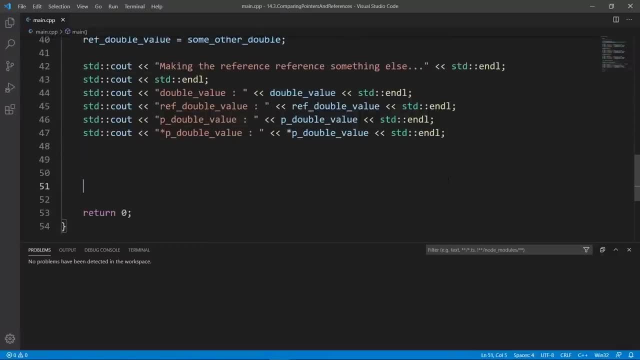 You're going to see that our pointer now is going to be containing another address. So what we can do is say pdouble value, which is our new pointer, and we're going to assign it the address of some other double value. And if we print the data now and go down, 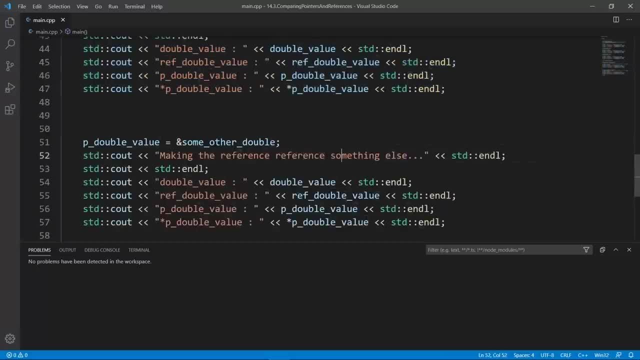 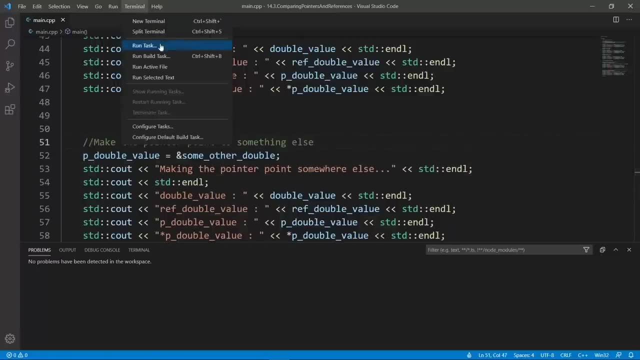 we are going to say: make the pointer point to something else. That's what we are doing here. And we're going to say the same thing here through a comma, And if we print this, try to guess what we're going to get. 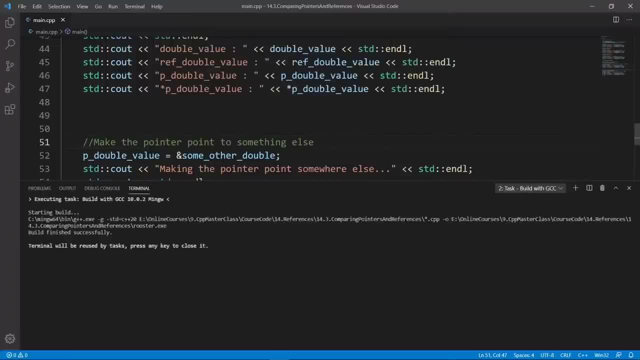 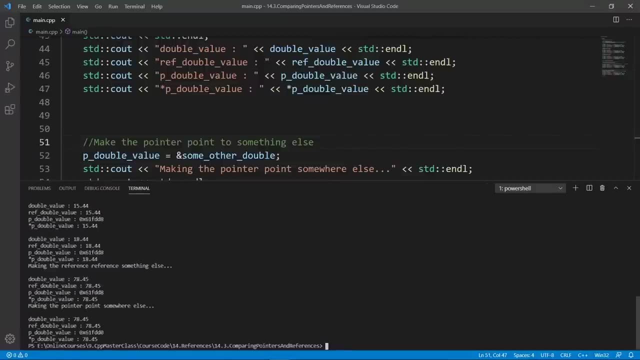 The pointer is going to contain a completely new address, because we can do that. We can make it point to somewhere else. Let's run Rooster And we're going to see our data here. Let's make sure we see the entire thing. 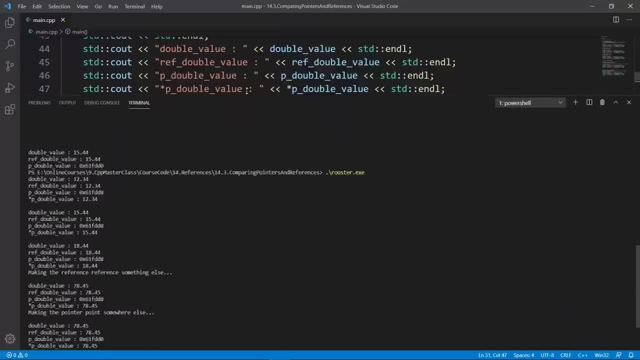 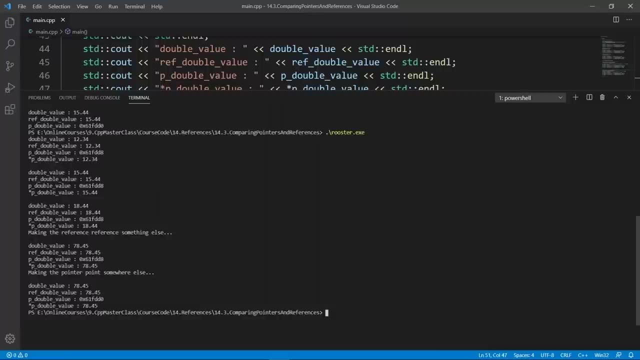 Okay, I think this is the data we have. Let's go up again. There's no harm in that. So we have our things that we have seen before. but what is going to be important here is that pdouble value now contains a new address. okay. 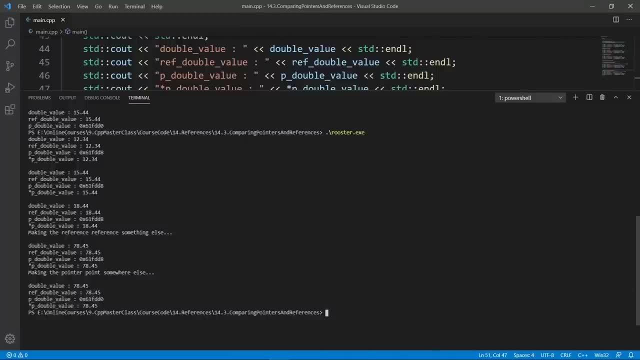 So this is really important and you have to understand that. So we made it. The pointer successfully points to something else and if we change the data in the pointer now, we're not going to be affecting the data we have in here. 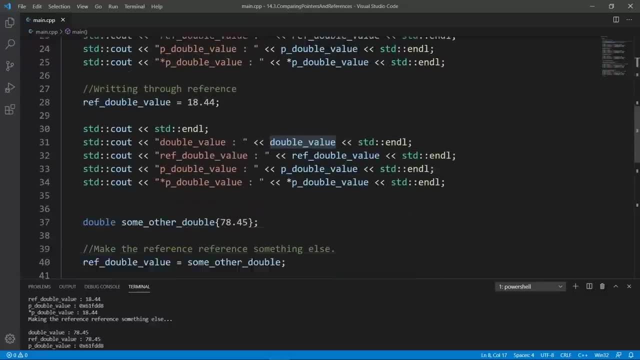 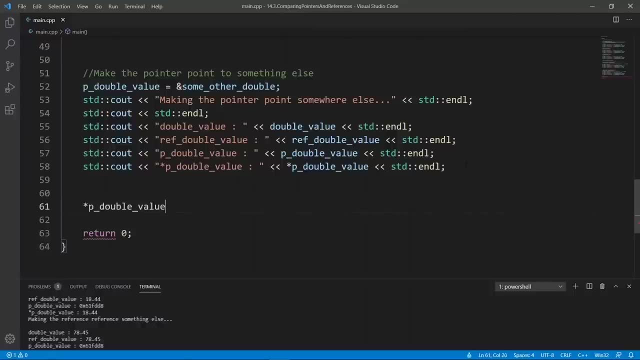 in double value. We're going to be affecting the data we have in some other double value here. Let's do that. We're going to change the data through the pointer, so we're going to say pdouble value and we're going to change this to 555.5.. 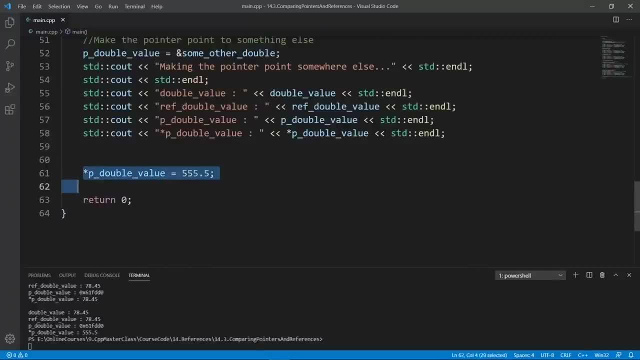 And now we can print the data and see that things have changed in memory And we're going to say we can print this to see the differences here. But before we do that, let's also print the address of the original variable and the address. 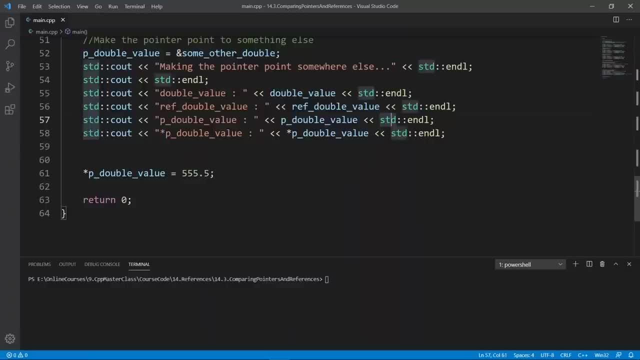 because for now we are just printing only the address through the pointer. So what we can do here is grab stdcout and say address of double value and we're going to put that out through stdcout here We're going to do that. 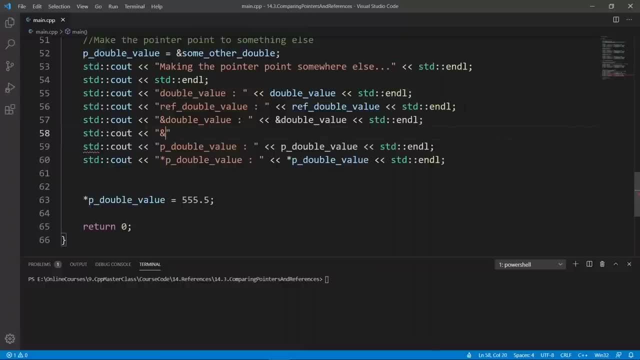 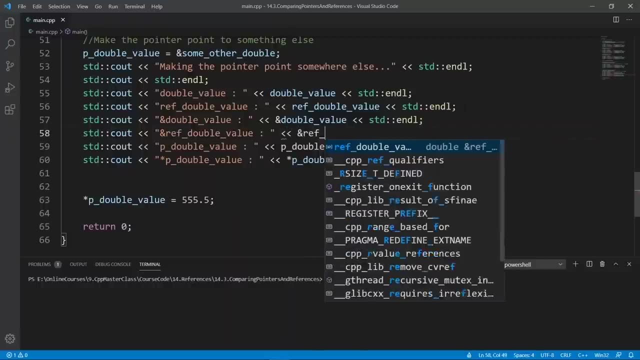 and we're going to print the address of the reference- Why not? So we're going to say address of ref double value, and we're going to put that out as well. We're going to say address of ref double value and we're going to say stdendl. 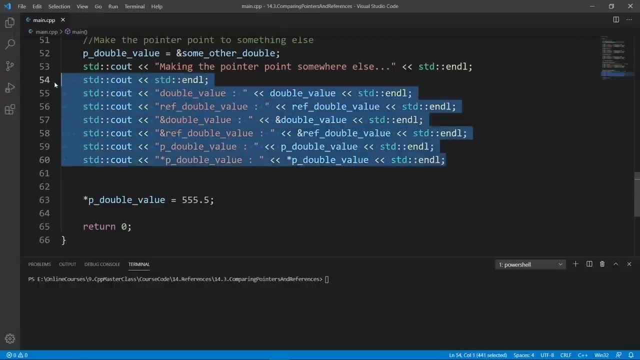 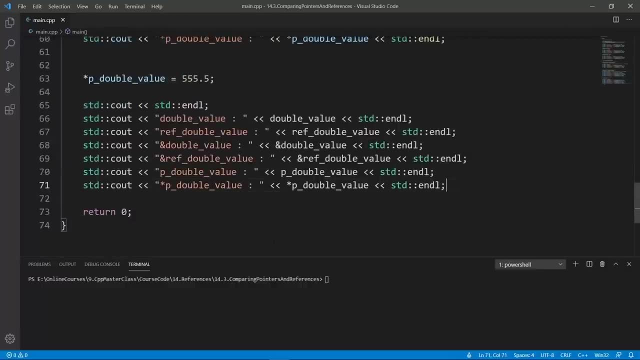 And after that we are going to grab the entire thing here and print it out after we modify the value in the pointer. I hope this is going to show things in a much more clear way. So we're going to build this with gcc. 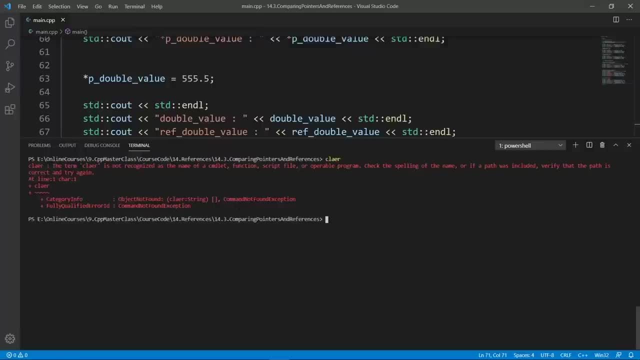 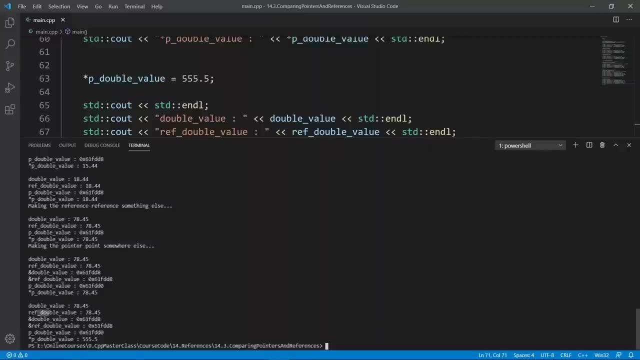 Let's do that. The builder is good, so let's clear and run rooster, And what you're going to see is that now the original variable is living at address here, which we can see in our reference. but the pointer now is pointing to something else. 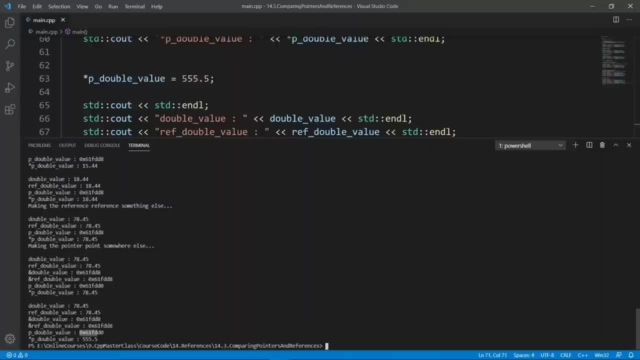 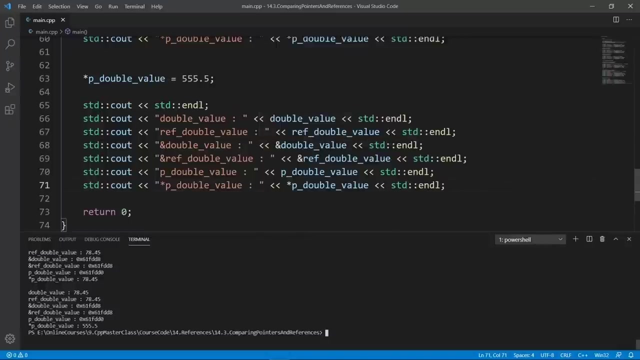 No wonder that the changes we did through the pointer are not being reflected in our double value, because these two variables now are living in different memory locations. I really hope you see that, And this is really all we had to share in terms of the differences between pointers and references. 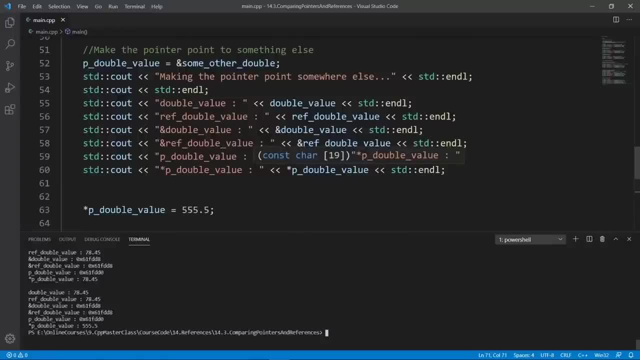 I hope you have a clear picture of what these two things are, And we are going to stop here in this lecture. In the next one we're going to see how the const keyword works with references. Go ahead and finish up here and meet me there. 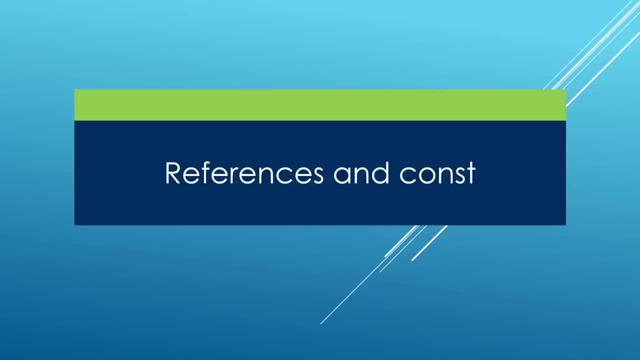 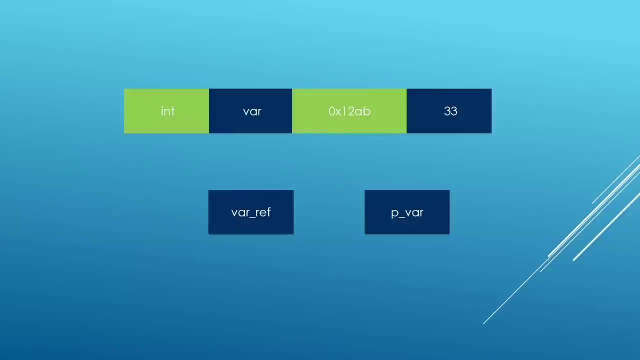 In this lecture we're going to see how the const keyword can be used with references And again the idea is to set up an alias to a variable and make it const So that we can't go through it to modify the original variable. 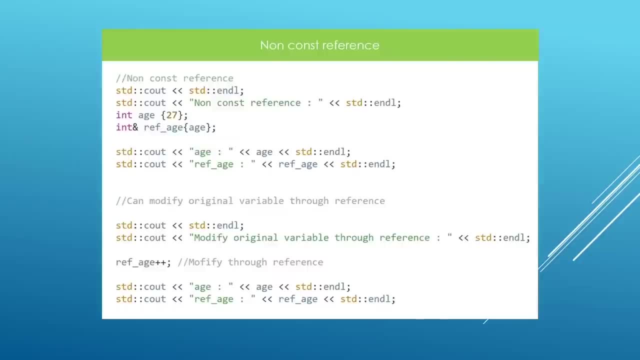 This is the syntax we use to set up a non-const reference that we have seen so far. So, for example, we can say int age, put in a value- 27 in this case- and set up a reference to age and initialize that with the age variable. 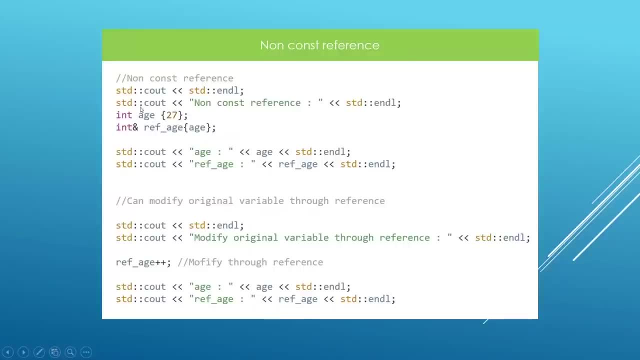 Once we do this, ref age can be used to modify this age variable here and whatever is inside. For example, we can go through ref age to increment the age and if we print the age now, we should get a 28 printed out. 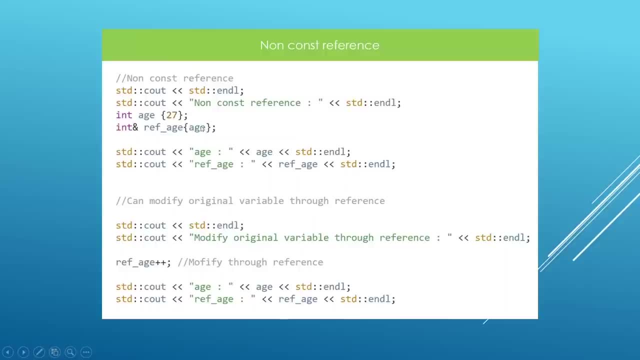 because this reference is going to change these two things at the same time, Or another way to say this: these two things, age and ref age- are referencing the same memory in your computer, So if you change one, the other is going to pick up the change. 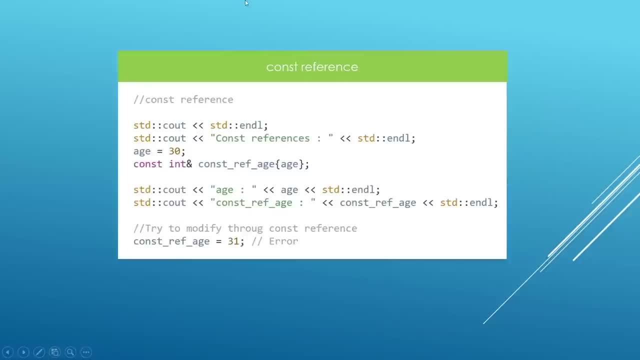 We can also set up a const reference and the syntax is ridiculously easy. You say const int reference like this, and your reference is suddenly const and you can't go through it to modify the original variable. If you need something like this in your application, 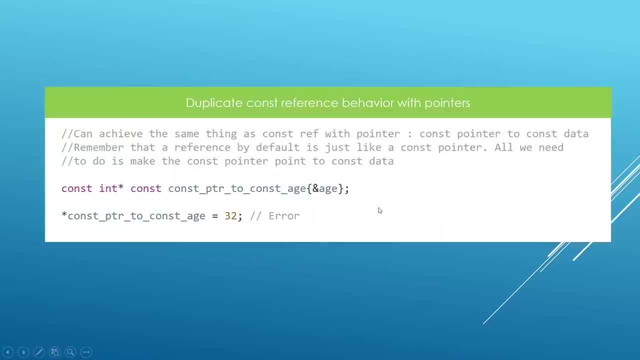 this is how you do it. You can also duplicate the behavior with count references, with pointers, and for that we can use a construct like const int, pointer, const. This is going to set up a const pointer to const which we can't use to modify the value that we are pointing to. 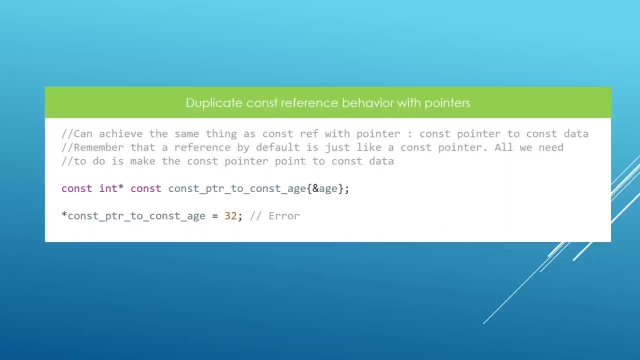 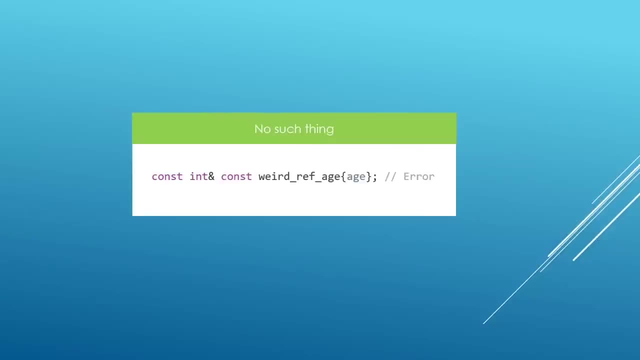 but it can also be used to point to something else. So this is going to simulate the behavior we have with references And you can do that if you want. And please know that we have no such thing as const int reference const. This is going to give you a compiler error because we have no such concept in C++. 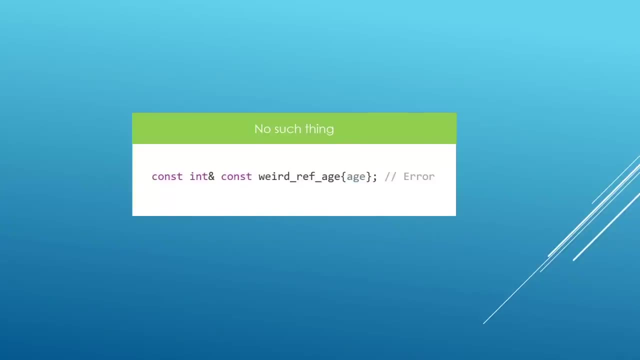 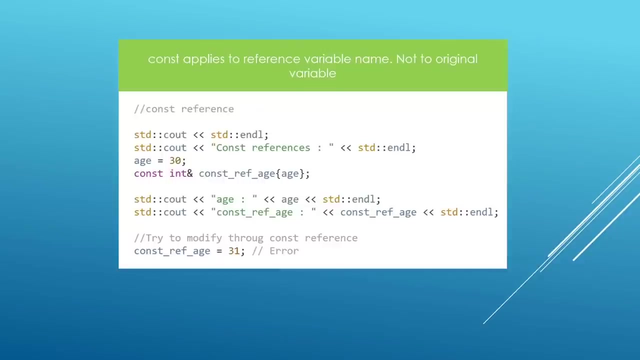 And my head is hurting right now trying to think about what this would even mean. And another thing I want to make clear before we head over to Vicious Video Code and play with us, is that the const keyword is going to apply to the variable name that you apply it to. 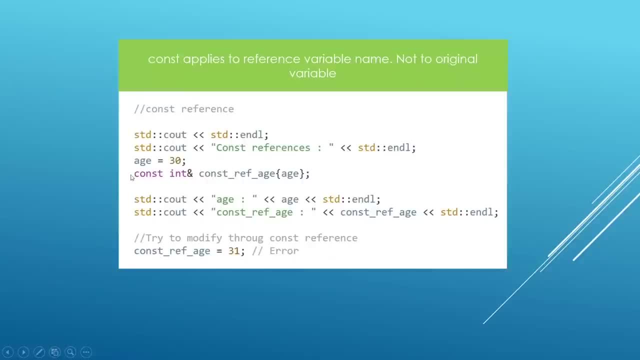 For example, here we have const reference age, which is going to be a const reference, but this doesn't mean that the age variable here has to be const. It can be const or it may not be const, but the const here applies to this variable name: const ref age. 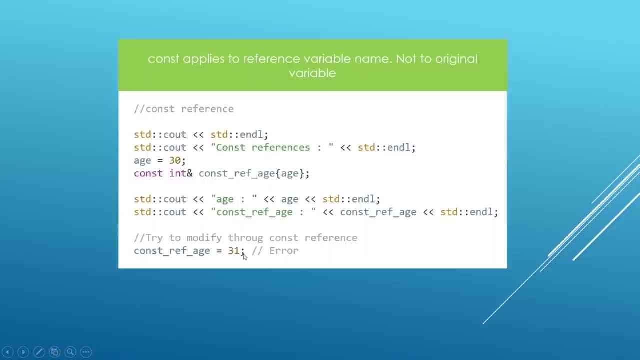 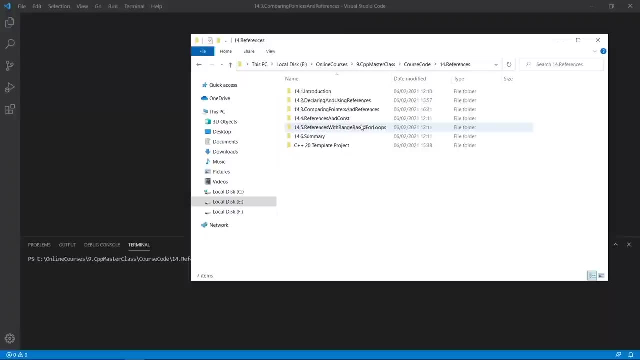 and we can't go through this variable name and modify the age. If you're trying to do that, we're going to get a compiler error. Now we can head over to Vicious Studio Code and play with us. Here we are in our working directory. 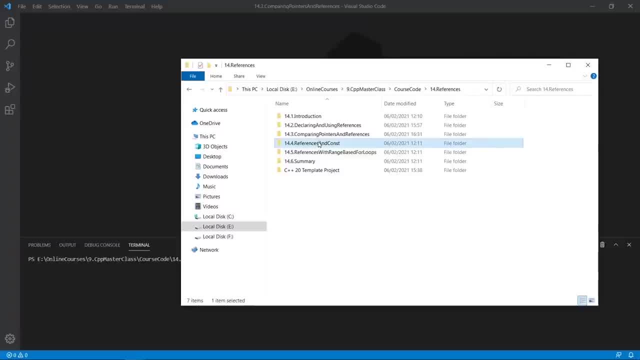 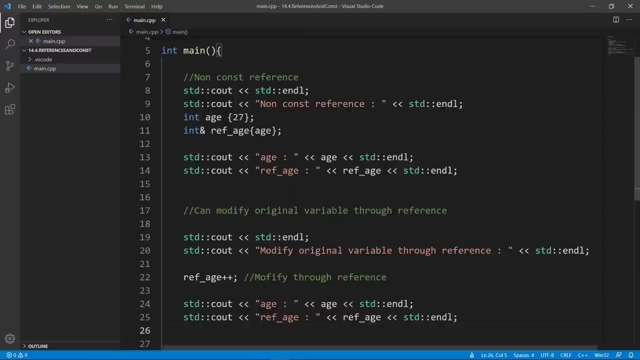 the current project is reference and const. We're going to grab our template files pretty quick- Let's do that- And we're going to put them in place. And we are going to open this in Vicious Studio Code. We are going to review the references we have seen so far in this little example here. 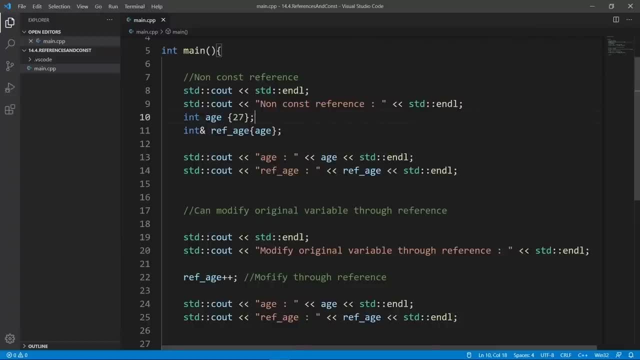 We have the age variable. It has a 27 inside and it is a net And we have a reference to it And this reference is not const, So we can go through this. This reference modified the age And if we do that, this is going to work. 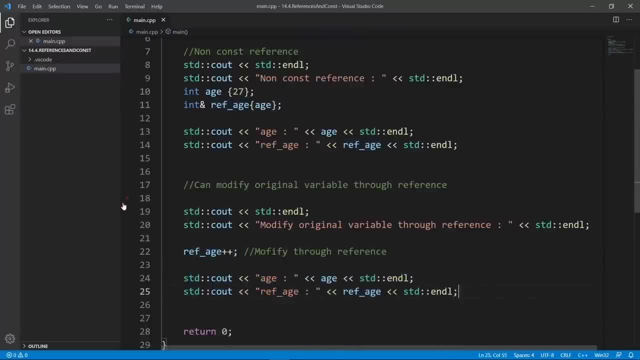 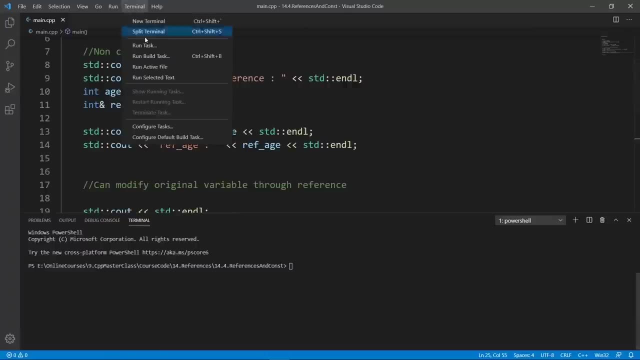 And if we print the age here, we're going to see that it has turned into a 28. And we can try and print this through the terminal so that you can see this for yourself. So let's run the task to build with GCC. 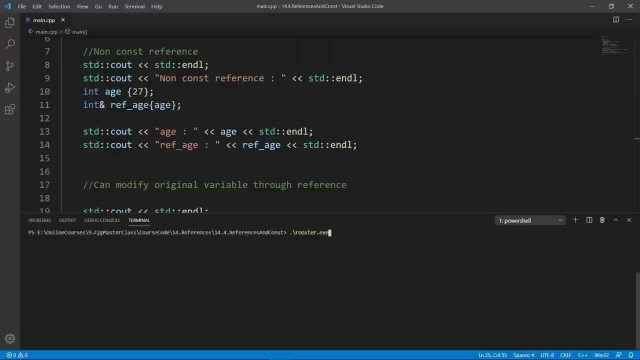 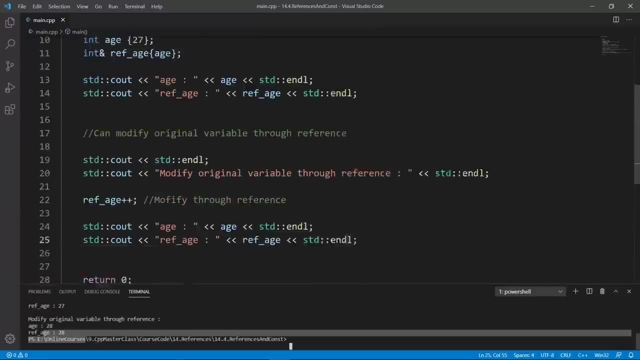 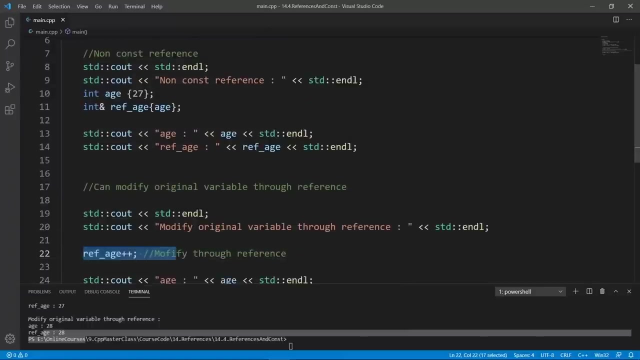 We are going to clear and run rooster And if we do that, you're going to see: age is 27.. Now it is 28. And we have successfully modified data Through our reference here. But if we change this reference to be const, we won't be able to do that anymore. 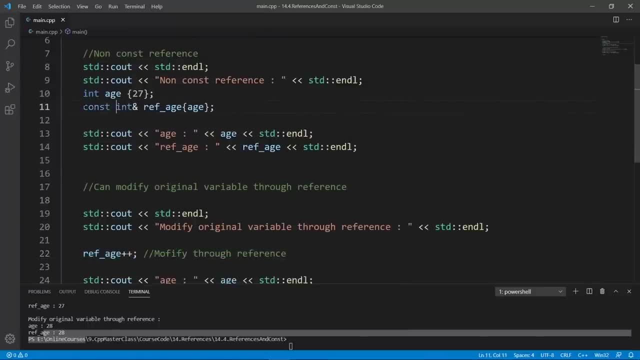 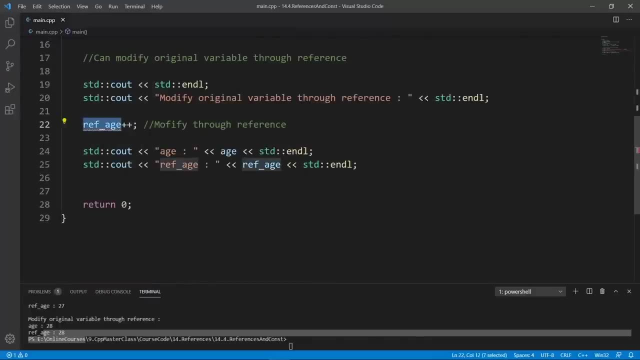 So let's try and make it a const reference. If we do that, we're going to get a compiler error. if we try to do something like this, Because this is now a const reference, We're going to go through it to modify our data here. 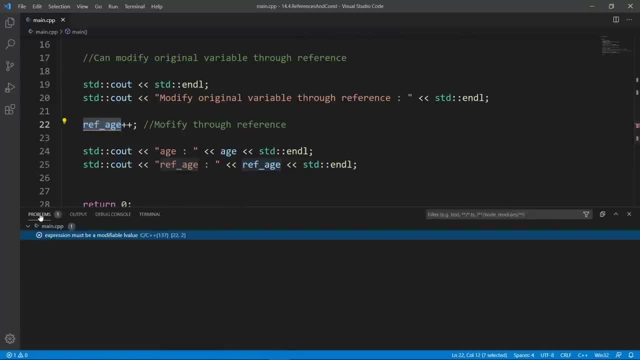 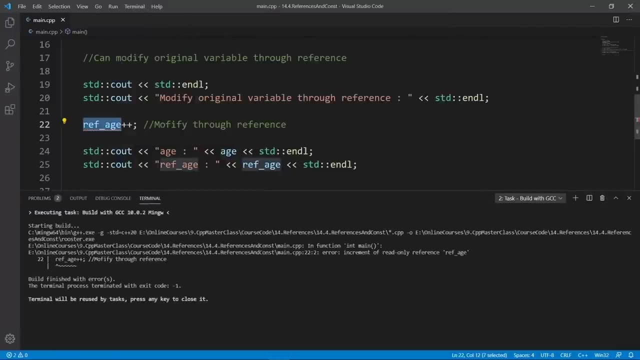 And we're going to get a compiler error Here. we have Vicious Studio Code complaining here, But if we ignore that and go through the compiler, we're going to see that we get the same compiler. We can't implement a read-only reference, which is this ref age here. 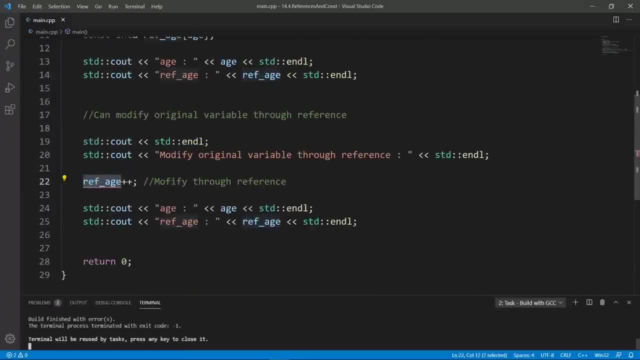 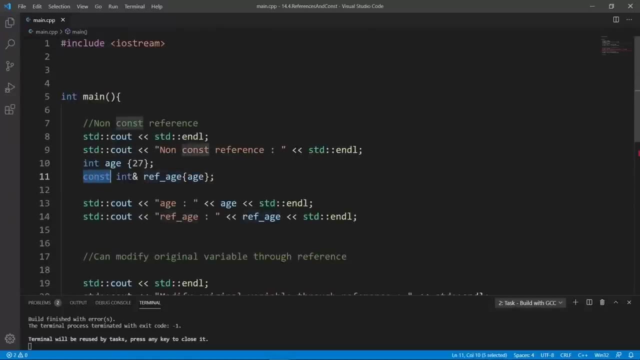 So this is what a const reference really is. You can't go through it to modify the data that is being referenced. And another thing I want you to really understand is that this const keyword here has nothing to do with the original variable. This is a const reference. 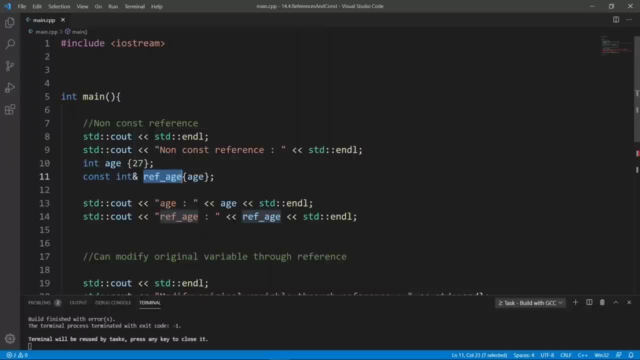 We can't go through it to modify the age variable. But this doesn't matter. if age is either const or not const, The constness here applies To this variable name here. So this const age may be const. If it's const it's going to work equally well. 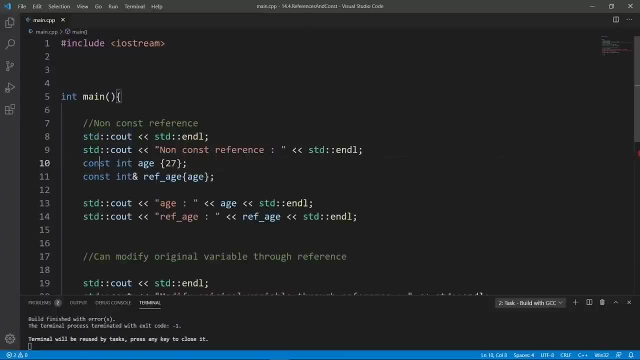 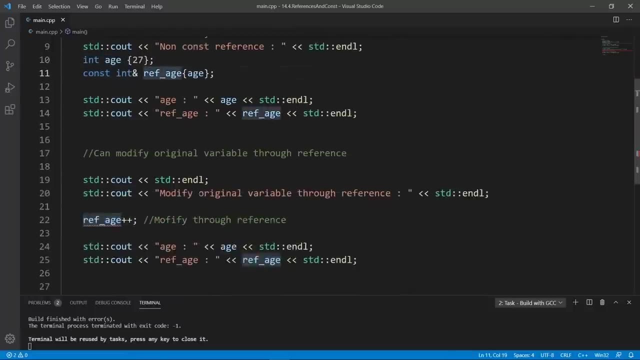 And we're going to still get a compiler error here. If it's not const, it's going to be the same. The const we have on our reference applies to this reference variable name here. This is what I want you to understand. Okay, this is what a const reference really is. 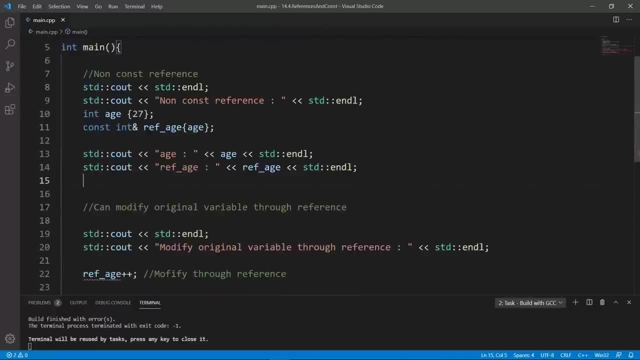 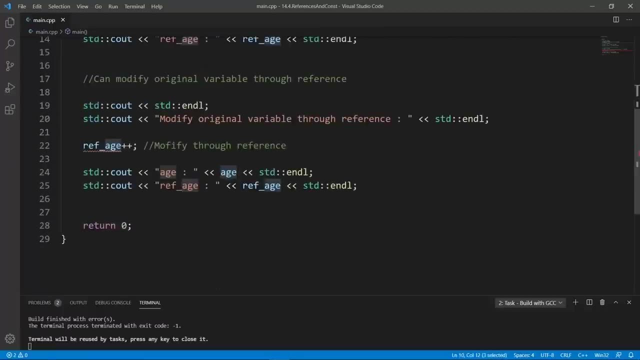 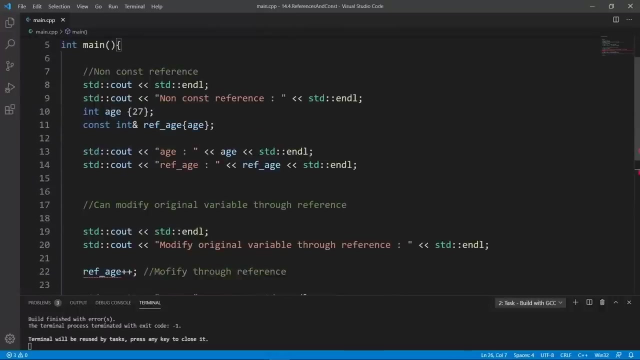 Another thing we want you to see is that we can simulate the same behavior with pointers. So let's set up a const pointer to const on this age here, And we're going to see that we can have the same behavior. But for that we're going to have to comment this out, because we don't want noise output. 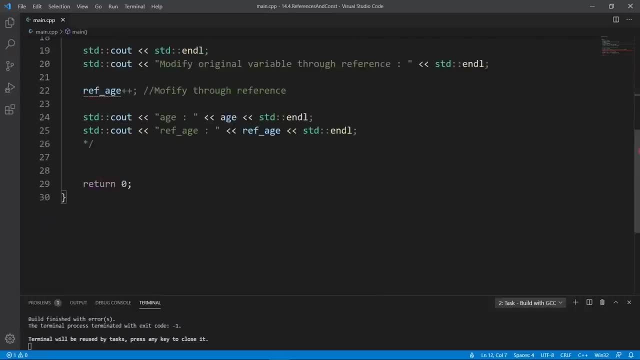 And we're going to go on top here and comment this out And say what we are intending to do. We can say that we are simulating reference behavior with pointers And the way we're going to do that, we're going to say const and pointer, const. 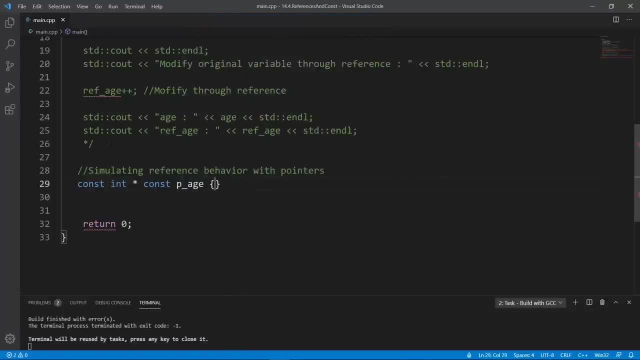 And we're going to say ph And we're going to initialize this With our age variable or the address of our age, to be super clear. Okay, so we have our pointer set up. Let's try and go through it and modify the age. 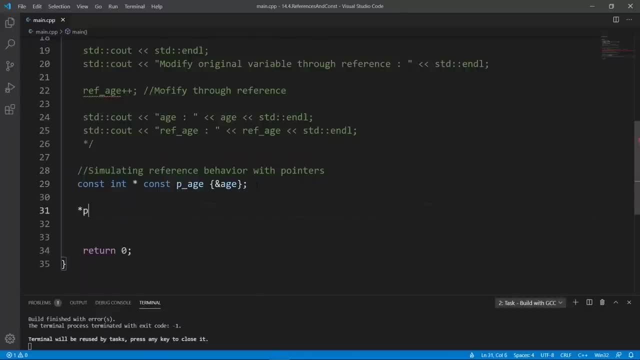 Let's see what happens. We reference- because this is a pointer- And we're going to say ph and say plus, plus, Or you can change this to another age, Let's say 45. And if we do this, we're going to get the same compiler error. 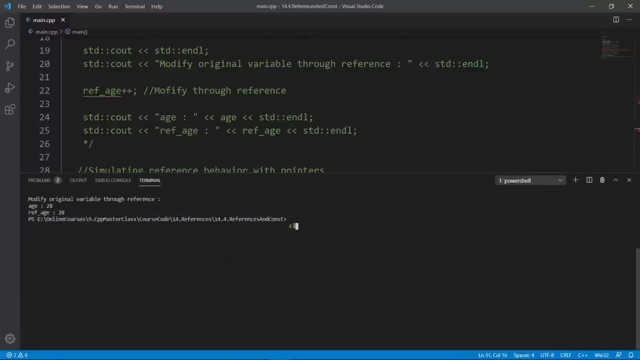 So if we build this- let's clear here, Clear, not clear, And I build again- We're going to get another compiler error Saying that we can't modify something that is read only. Assignment of read only location. This pointer can't be used to modify the data in this age location here. 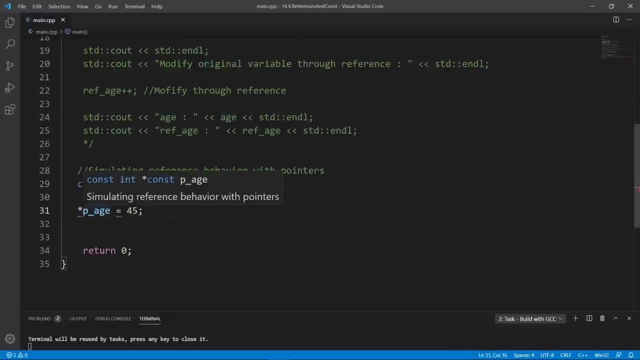 So this is the same behavior with references. Because the reference by default can't be made to point somewhere else, We had to make this pointer also a const pointer, preventing us from making it point to other locations. So this is how you can simulate references with pointers. 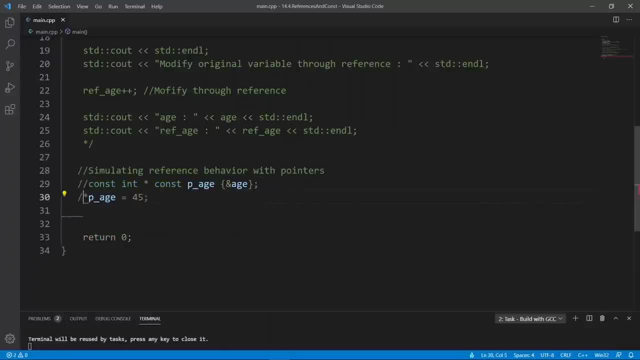 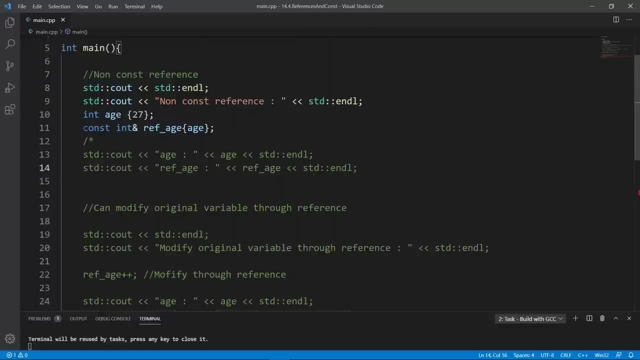 And this is really all we set out to do in this lecture. I hope you found it interesting. The main idea was to let you know how you can work with const references And once you have the const reference, you can't go through it to modify the original data. 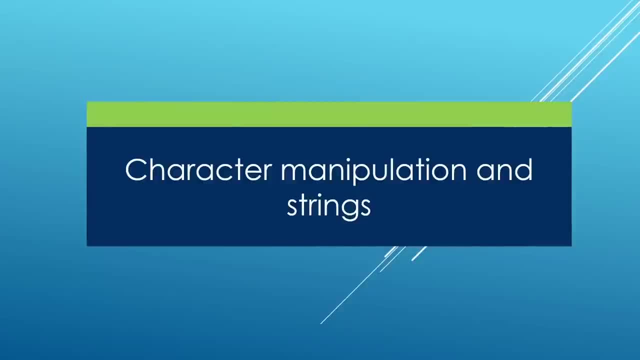 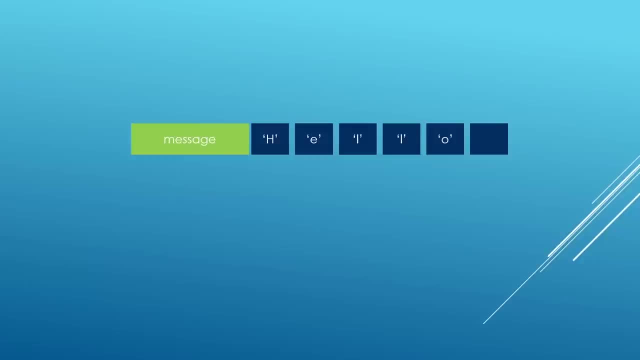 If you do that, you're going to get a compiler error. Welcome to this new chapter, Where we will be doing cool stuff with text data. Yeah, We have seen that we can model a character array and store in a bunch of characters, and we could, for example, 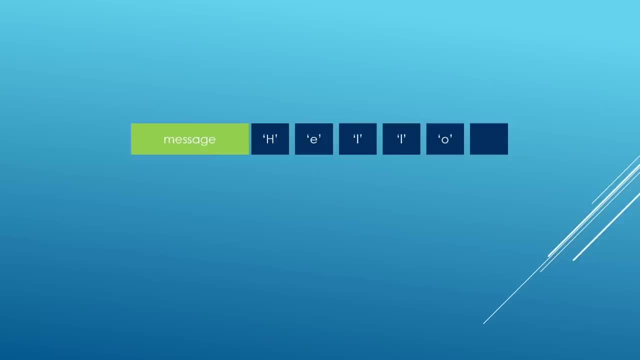 call this character array message and manipulate it in memory in this structure. we will see that this is actually the way text data is stored in c plus plus, and we have a lot of facilities built on top of this character array construct to make it easy to work with text data. we will see that. 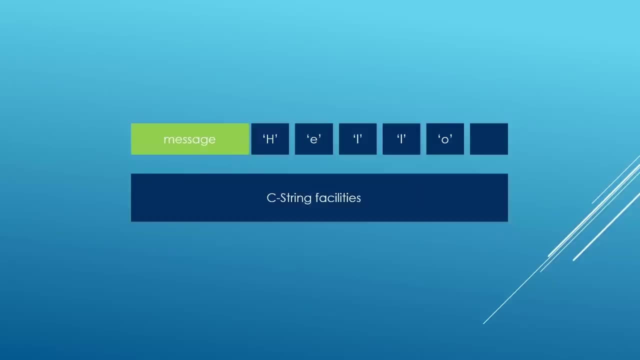 we can use character arrays to model c strings which are a facility we use in c plus plus to handle text data, and we will see that there are a few welton facilities we can use to manipulate that. we can get the length of the string. we can concatenate strings and put them together. 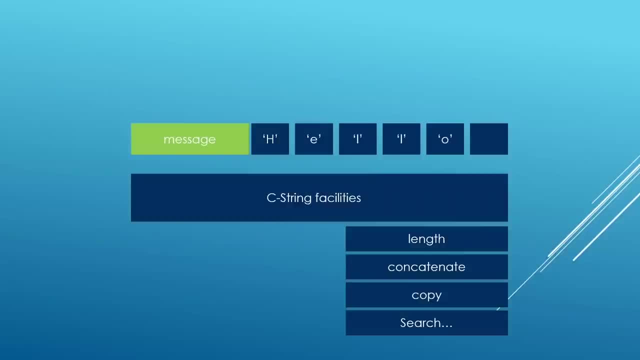 we can copy strings, we can search for data inside strings, we can do all kinds of crazy things, but we will see that c strings are not that easy or convenient to work with. for example, you need to keep track of how big the string is in memory. you need to also remember to make sure it ends. 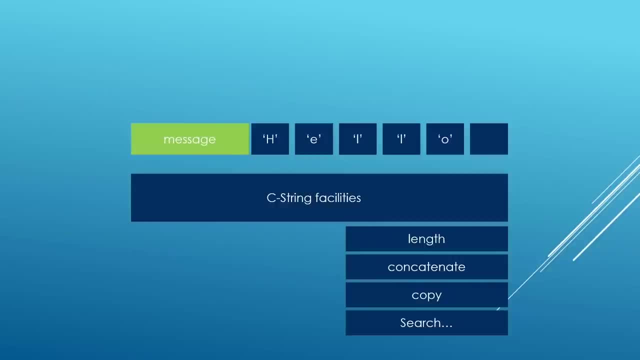 correctly and we will see the details about that in this chapter. long story, short c strings are not safe or convenient to work with in c plus plus, and c plus plus provide another type that really boils on top of character arrays, but it gives us an easier interface to work with and we can. 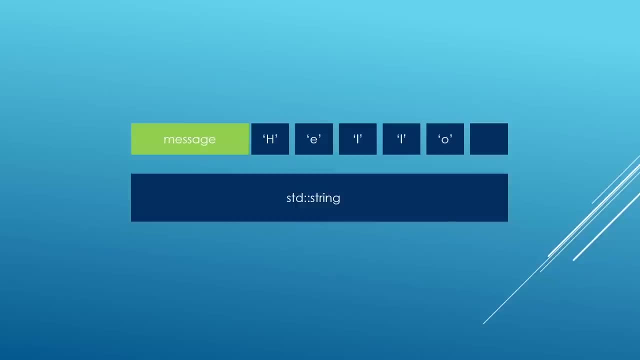 just focus on storing in the data and doing stuff with it, and it is very easy to work with this kind of thing. so I hope you can see the details about this in this chapter in our c++ programs and the big idea about what we're going to be doing in this chapter. 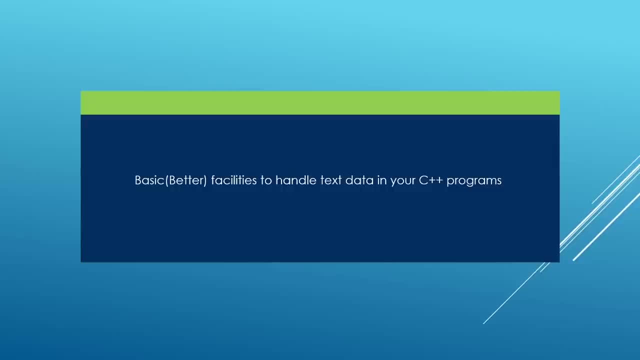 is learn about the facilities we have in c++ to handle text data in our c++ programs. in the next lecture we're going to start and show you how you can manipulate individual characters in a character array. go ahead and finish up here and meet me there. in this lecture we're going to be 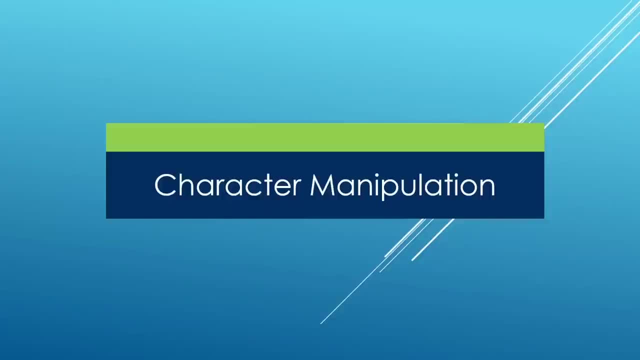 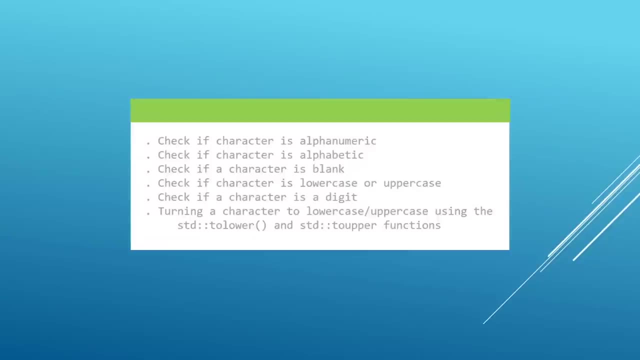 learning about some facilities in the c++ standard library that can help us manipulate characters, and here are a few things you might want to do with those facilities. for example, you might want to know if a character is alphanumeric or if it's a number or a character. you might want to know if 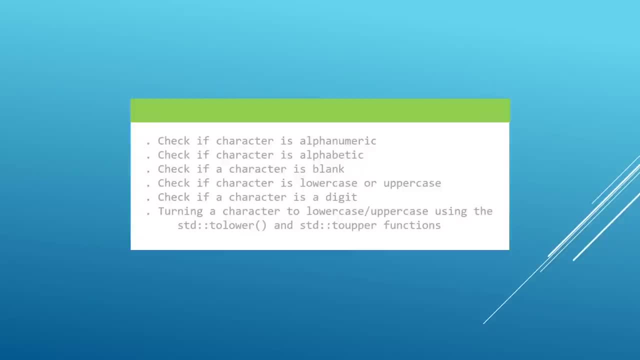 it is alphabetic, you might want to know if it's a blank character. you might want to know if it's a lowercase or uppercase character, depending on what you want to do in your application, of course. and then you might want to know if it's a number or a character you might want to know. 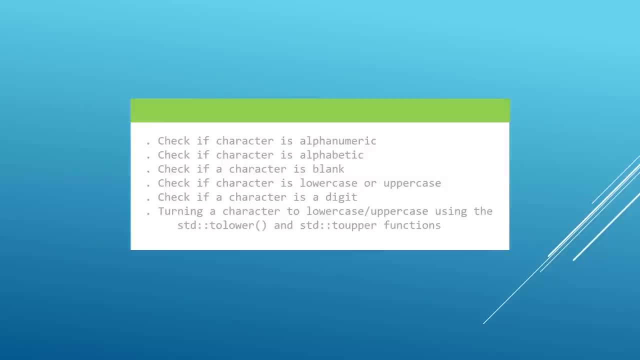 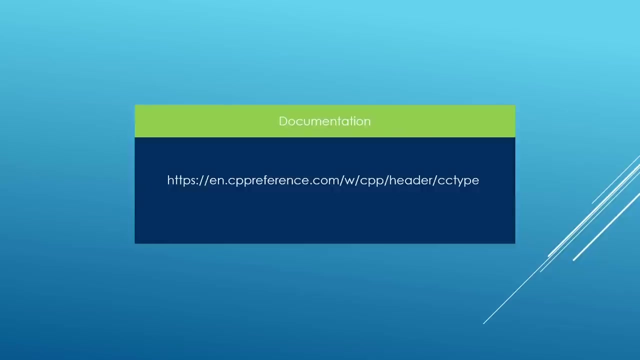 there are facilities to check if characters are digits. there are even those that help us. you know, transform characters, make them lowercase or uppercase, and we're going to see these examples here. all of these are documented at cppreferencecom so you can go there and find the. 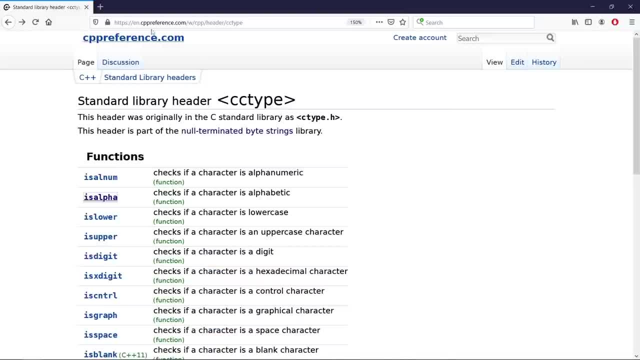 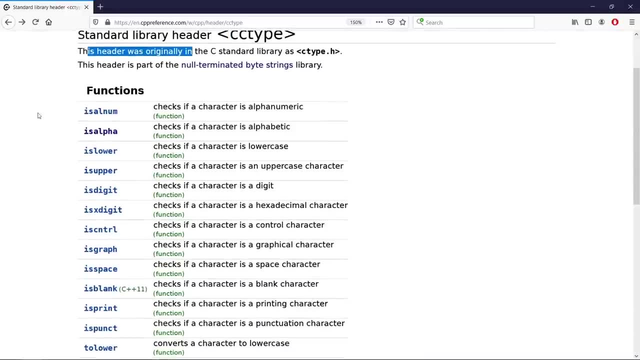 documentation. here is the same link opened in my browser. you see that they live in the cc type library, so you need this included if you want to use them. and you see that there is quite a bunch of them. we are going to cover just a section of them and i 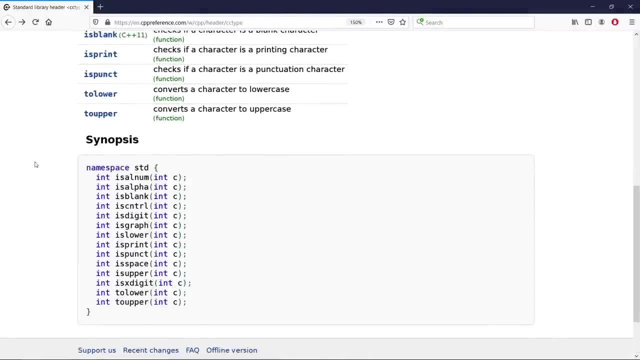 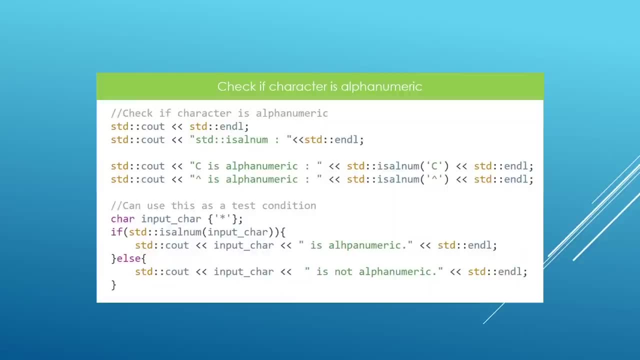 will leave you to use the documentation if you need to use any more of these guys. our first example here is going to help us check if a character is alphanumeric and the function we're going to use from the c++ standard library is std, is l, num, and you just pass it a parameter of. 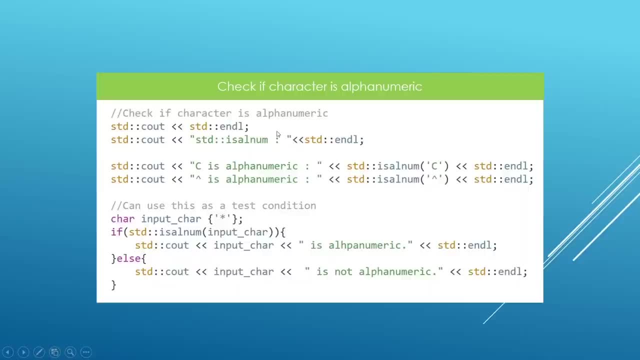 a character and it's going to tell you if a character is either a number or a character alphanumeric, or if it's not. if it is alphanumeric, you're going to get a value that is different from zero, which can be treated like a true. if it's not, you're going to get a value that you can treat. 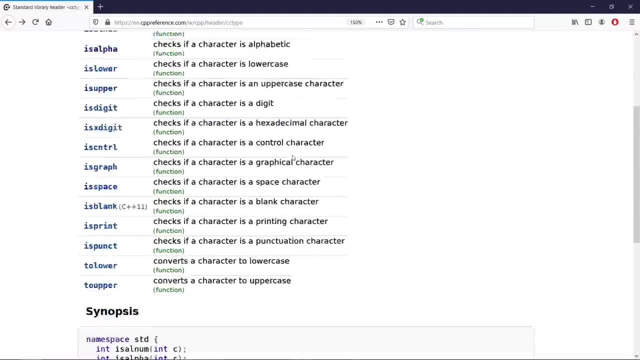 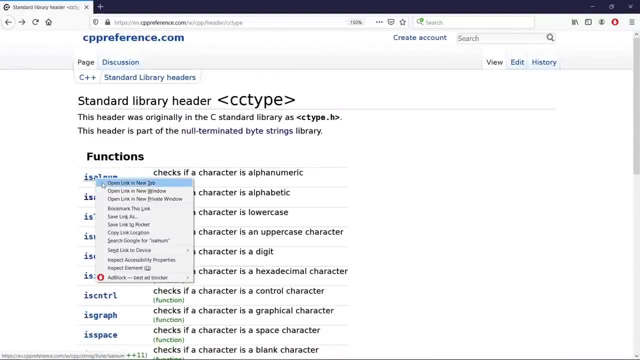 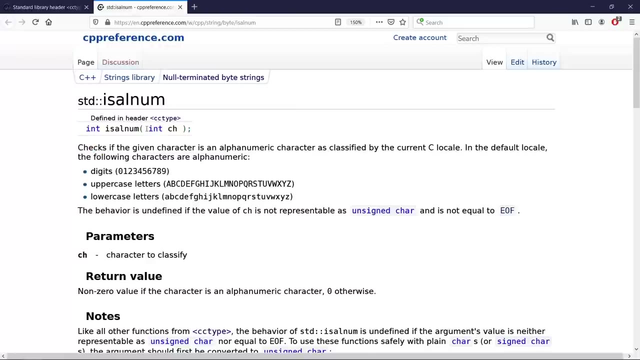 like a zero. and how do i know this? well, we can check the documentation. so if i come back to our link here and there is a function here is al num, i can open it in another tab and it is going to tell me what this function does checks if the given character that you pass as a parameter here. 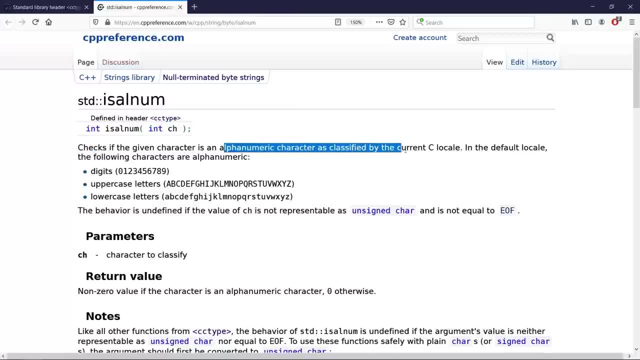 is a number of characters that you pass. as a parameter. here is a number of characters that you can call in alpha numeric character as classified by the current siloca. so it's going to tell us if the character is alphanumeric or not. you give it a character and what you get from that is the return. 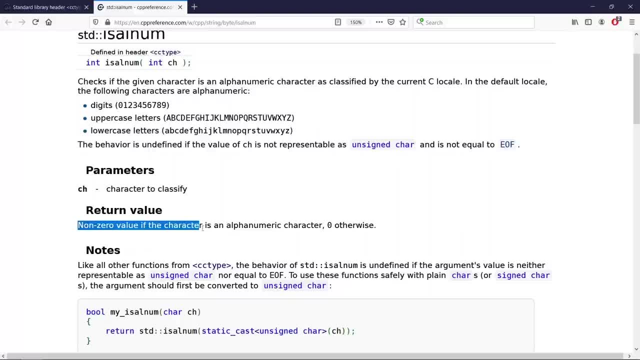 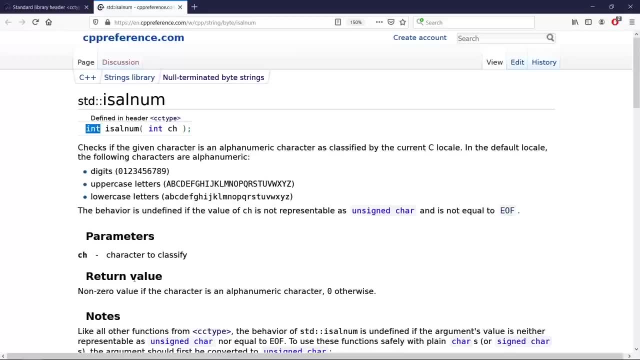 value. here it's going to return a non-zero value if the character is alphanumeric. so this non-zero value, which is an integer, because that's what we get out of this function- is going to be treated like a true. and if this character here is not alphanumeric, then it will not be treated like true. 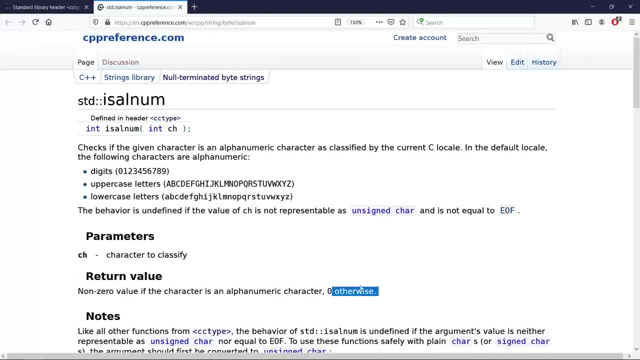 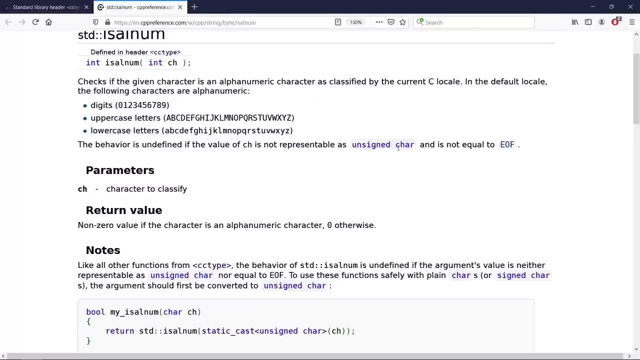 alphanumeric, we're going to get zero that we can treat like a false. this is really cool and if you go down here, you're going to find a few examples. i don't want you to worry about this c locale thing. it is a setting that allows you to say more about the meaning of the characters that you are storing. 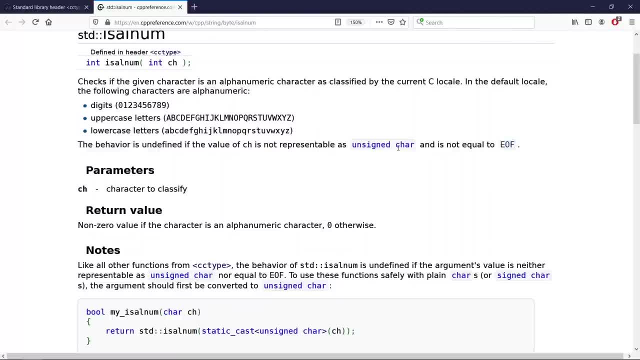 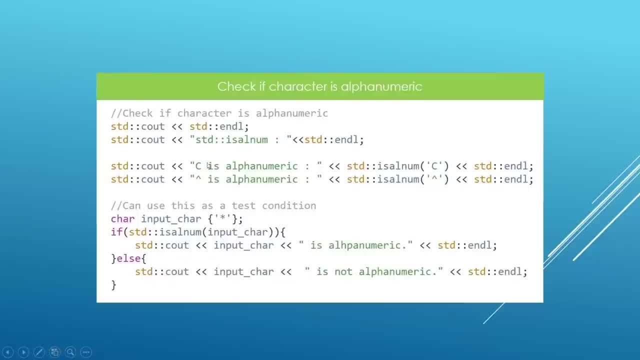 in memory. but for now we're just going to be happy with the defaults and use this function as is. it is going to work enough. well, okay, here is our function again. so here c is alphanumeric. we expect to get a value different from zero because c is alphanumeric. and the second example here is not. 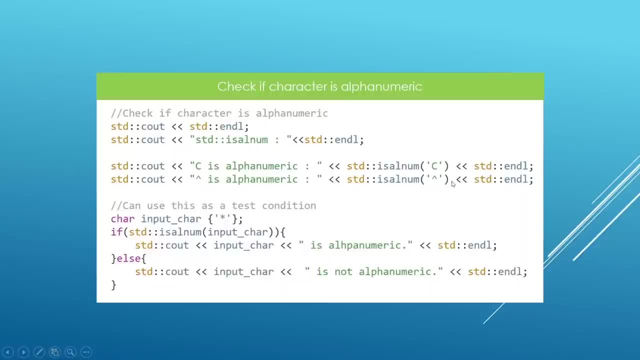 alphanumeric, so we expect to get a value that is equal to zero and we can use the return of this function in a test. for example, we can say a character we put in a star here it is called input car and we say f is al num and we pass this character. 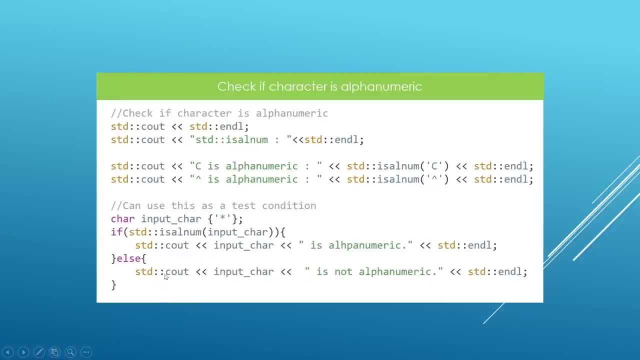 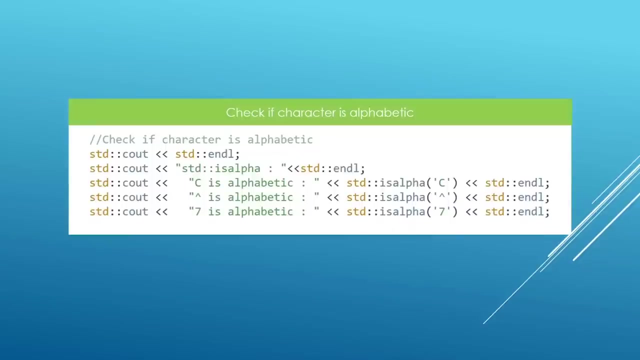 we're going to print out this character is alphanumeric. if it's not, we're going to print is not alphanumeric. you can do that and you can do all kinds of crazy tests in your c++ applications. here is another example that we can use to know if the character is alphabetic. so it's going to. 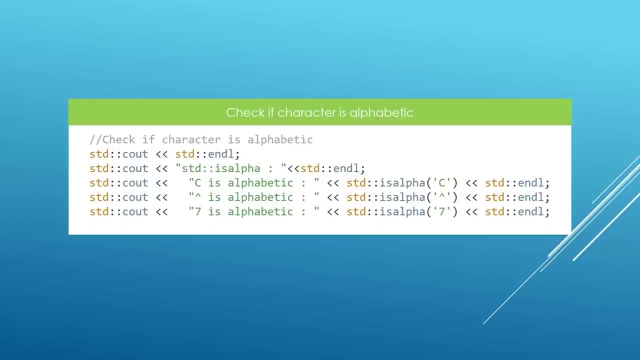 return a value different from zero. if the character is a- an alphabet character- a through z- that's going to return something different from zero. and if we pass something that is not, for example, this second line here or the seven at the third line here, we're going to get a value equal to zero because that's not alphabetic. we have another facility to 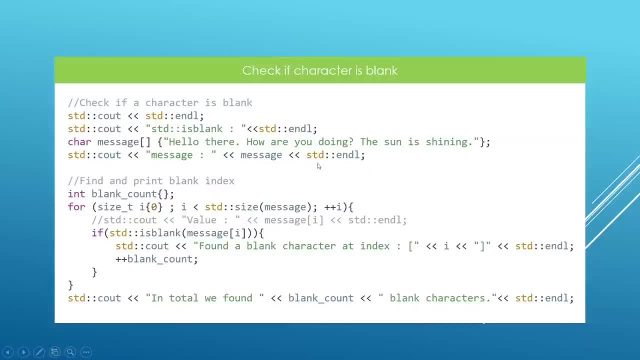 help check if a character is a blank character, and we see an example of that here. we have a character array called message. we have a couple of blanks inside and we can hunt for them using the is blank facility from the c plus plus standard library. here we have a variable. 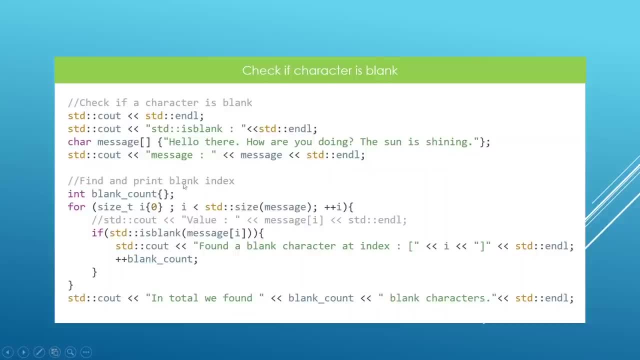 that is going to keep track of how many black characters are in. here it is initialized to zero and we're going to loop around. okay, and we're going to loop by the amount equal to the size of the message array. here we can use std size again, because this is a row array, it is a static. 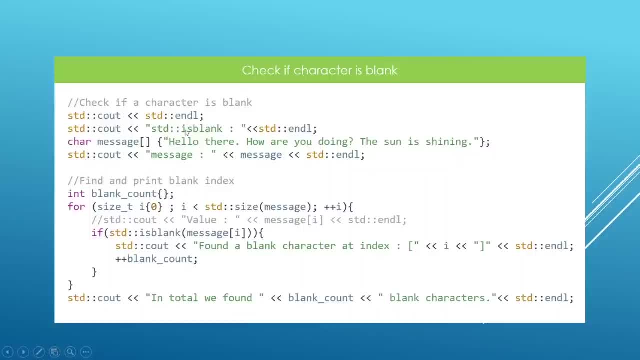 array and we can use std size. it is going to give us how many characters we have in this array. you already know this and if we get inside, we are going to try and check and see if the current character is a blank. if it is, we're going to print that out and we're going to increment our 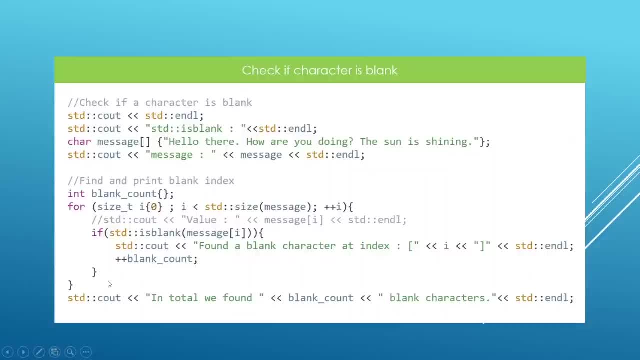 blank count. by the time this loop is done, we will have printed out a lot of blank characters- if we happen to have them in our message- and at the end we're going to say: in total, we found however many blank characters. this is what we're going to see if we run this program and hopefully you can see. 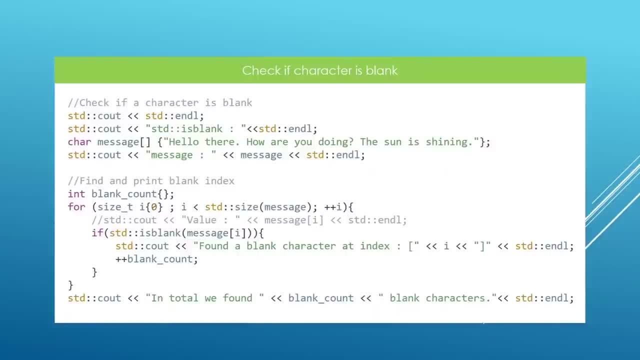 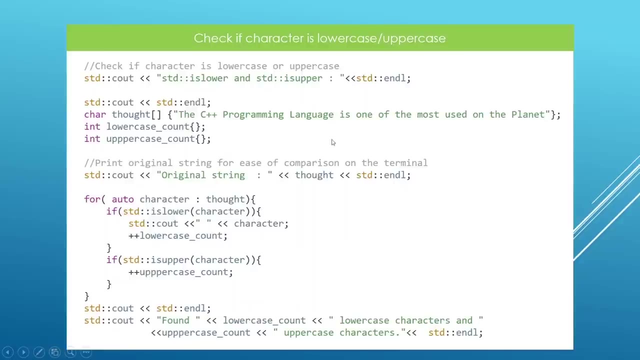 how useful this can be in text processing applications. if that happens to be what you are working on, we're going to run this example in visual studio code in a minute. here is another example that we can use to check if a character is uppercase or lowercase. we have an array of characters here. inside we have some text and we have a few. 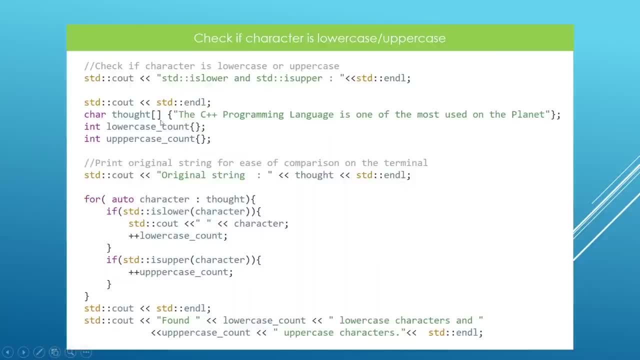 variables to keep track of how many characters are lowercase or uppercase. we're going to set up a loop which is going to be a range based for a loop and we know that through std is lower, we're going to increment the lowercase count if it is uppercase. we're going 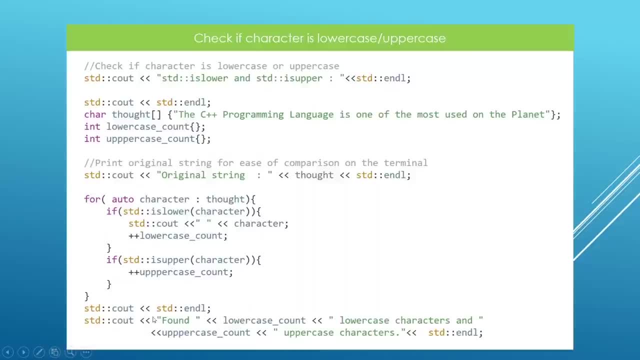 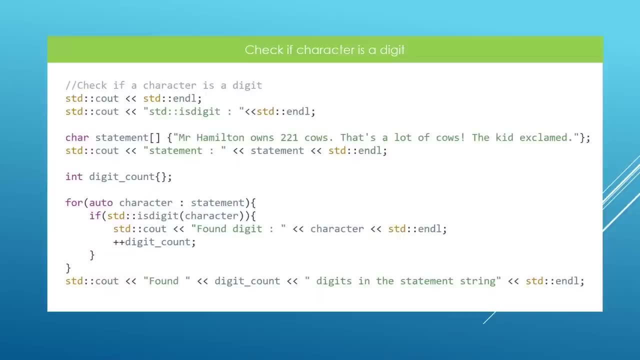 to increment the uppercase count. this is how we can do this, and we are going to print that information when the loop here is done. okay, we still have a few examples ahead. the current one is going to check if a character is a digit. if you want to do that, you can use this, and we have 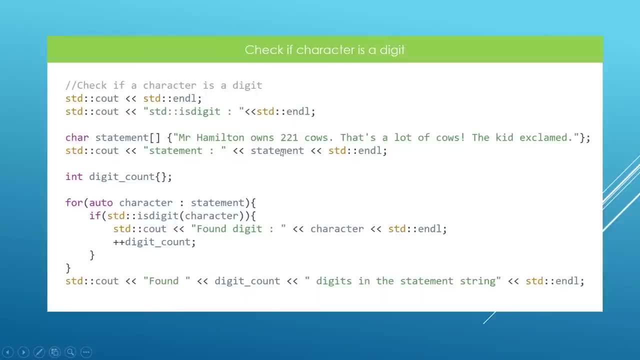 a character array here and we're going to have four digits inside this message here. so we're going to do basically the same thing. we're going to set up a variable that is going to keep track of how many digits we have in this message. we are going to loop around using a range based. 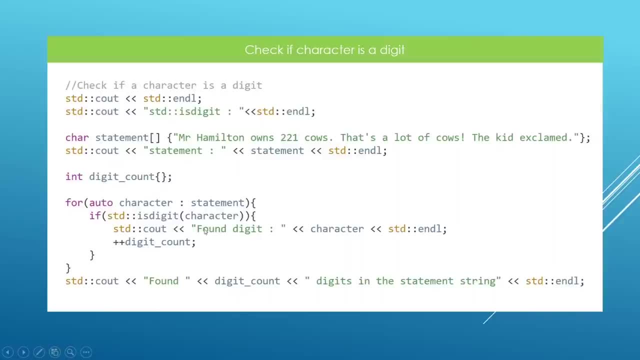 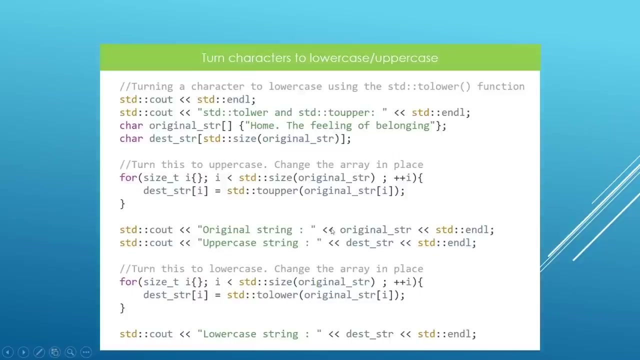 for loop. we're going to check if the current character is a digit and we're going to increment our variable here if it happens to be the case, and at the end we're going to say how many digits we found in our message here. it is this simple. the last example we're going to look at. 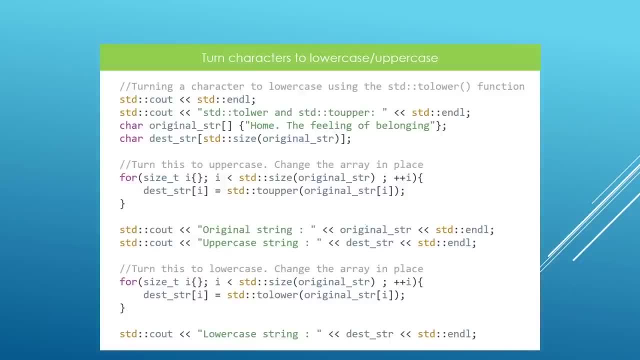 is to help us turn a character into lowercase or uppercase, and here is an example that is going to help us play with us. we're going to have a character array called home, the feeling of belonging, and we will set up a destination character array that we're going to store. 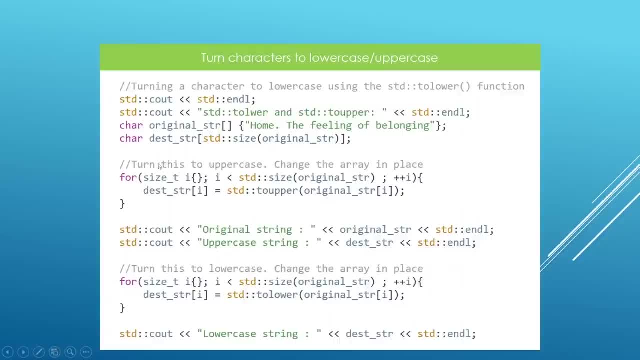 whatever we want to set up in here, you see a loop that is going to turn our message here into uppercase and you see we're going to loop around by this amount- the size of original string- and we're going to be grabbing each character at each iteration. 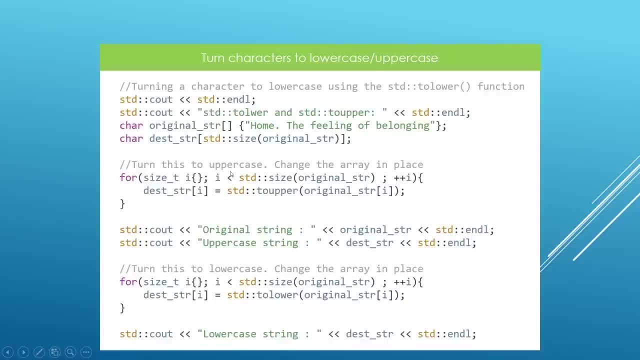 and turning that to uppercase. this is what std to upper function does the researcher of. that is going to be stored in our destination string and by the time we are done here, original string is going to be however it was, but uppercase string is going to be stored in our destination array. 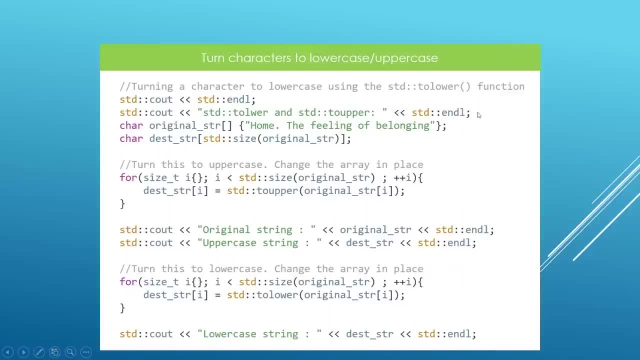 and if we print it out, we should see this thing printed in uppercase. we can basically do the same thing and turn the string into lowercase, and our destination string is going to be now lowercase, and you're going to see that this works out pretty well now that you have a basic understanding about how these things work. 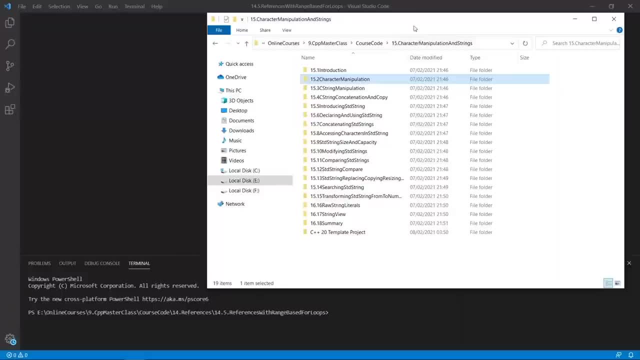 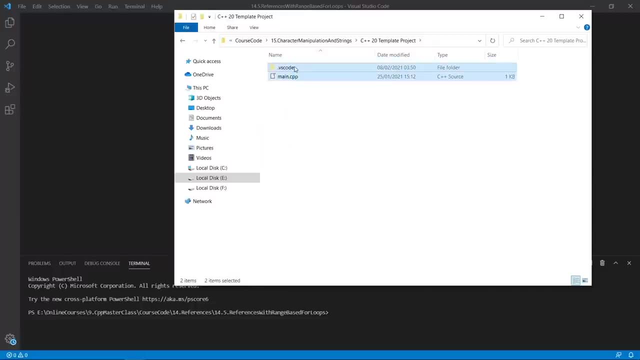 we're going to head over to vg studio code and play with us. okay, here we are in our working directory. the current project is character manipulation. we are going to grab our template files, like we always do, and we're going to put this in place and we're going to open this in. 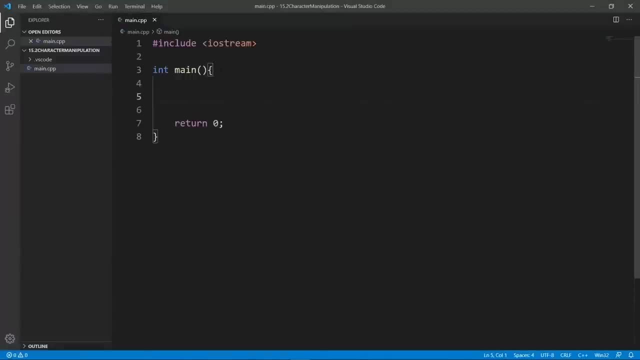 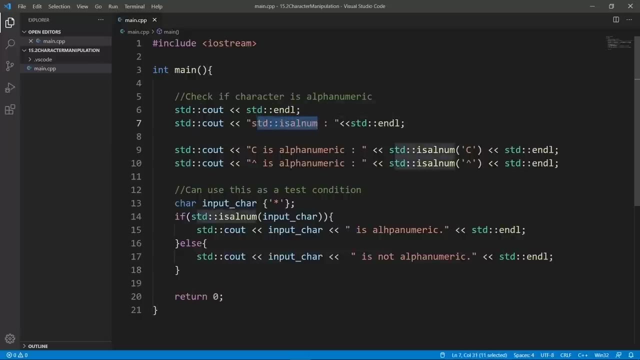 visual studio code pretty quick and we are going to go down and put in our first example. this example is going to be using the std is lnum facility and this is going to be checking if a character is alphanumeric. we're going to see what we get from this if we print this out. we're going to check if. 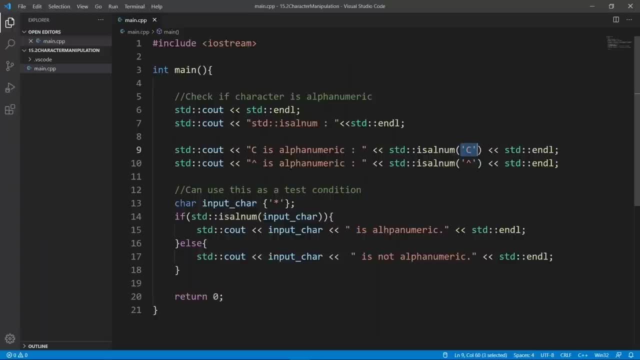 c, the character c is alphanumeric. we're going to see what we get and we're going to check if this- here i don't know how to pronounce it, i'm sorry- we're going to check if it is alphanumeric. we're going to see that and we're going to use this in a condition. we're going to check and see if. 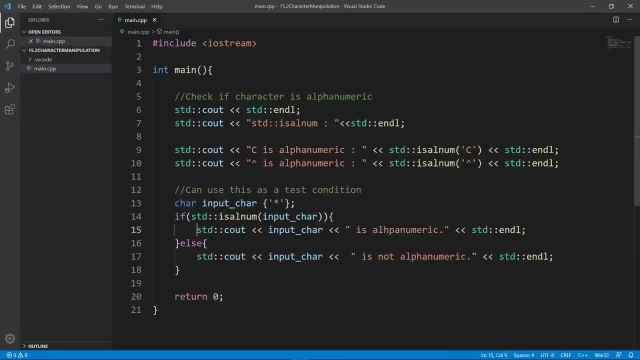 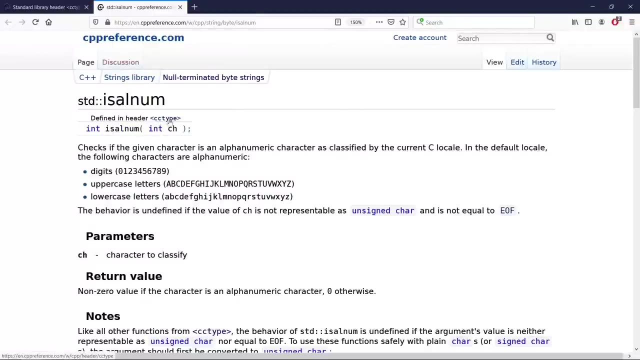 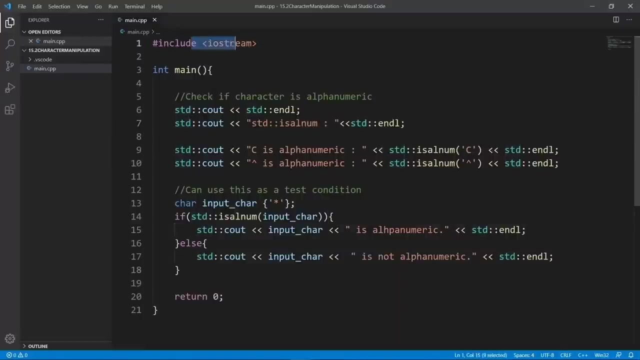 our star character here is alphanumeric and we're going to print that out. we're going to say it is alphanumeric or it is not. from the documentation we know that this thing lives in the cc type library so we may want to include that, but it is possible that it is coming from iostream here. 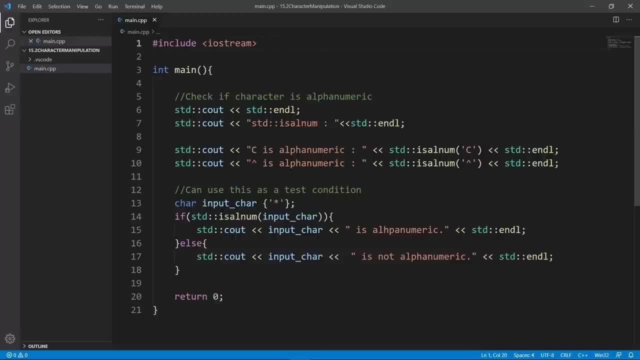 that's why we don't see visual studio code complaining here. as an example, if we try and comment out this include here, you're going to see that this is not going to make sense anymore. okay, so the include needed to use these guys here is coming from iostream. okay, so we're not. 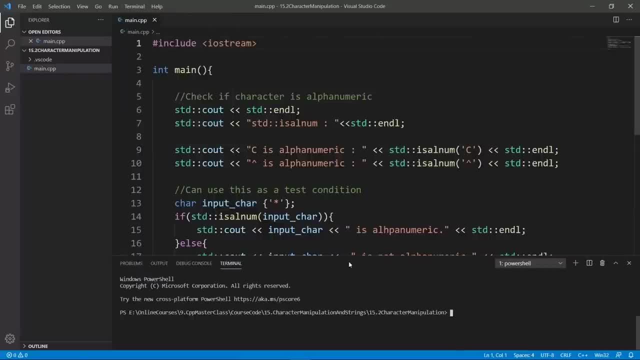 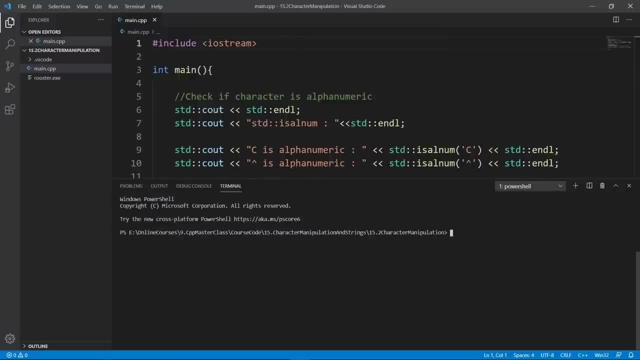 going to include that here. we are going to open up this visual studio code and we're going to a terminal and build this with gcc and you're going to see that the build is good. if we go down and clear- let's clear properly- and run rooster, we're going to see that c is alpha. 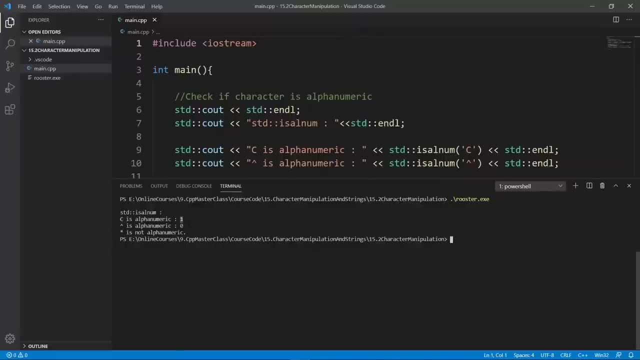 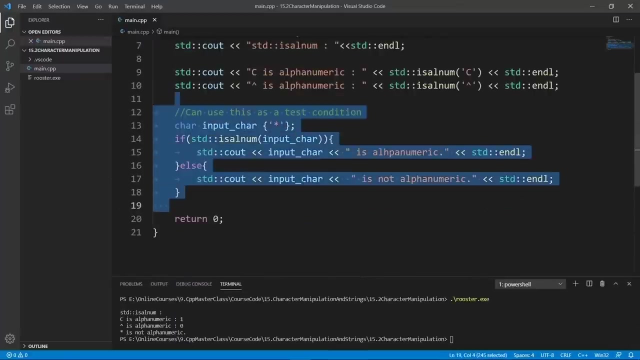 numeric because we have a one. the one can be treated like a true and the character here is not alpha numeric because the result is zero. and you see that the star here is also not alpha numeric, and we know this through our test here, and you see that we can do things like this with 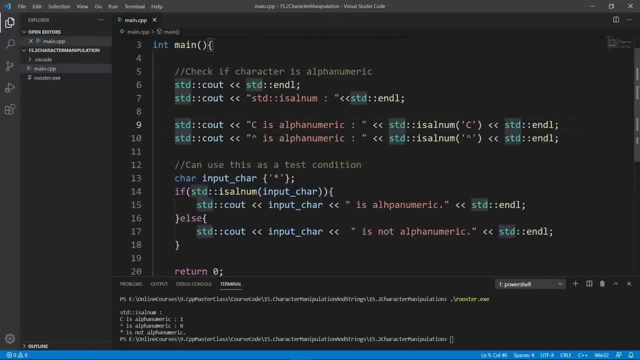 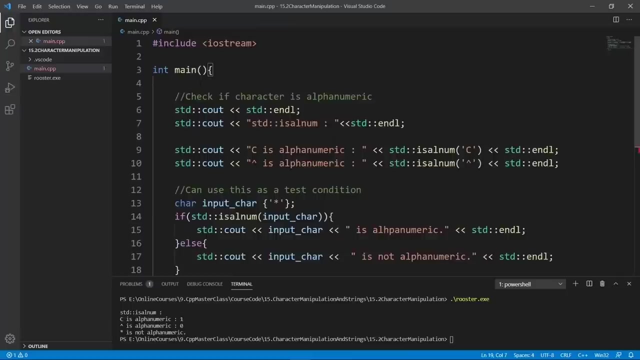 this facility here. if you want to get true or false from this function, you cannot turn this into booleans using static casts, but we're not going to do that here. you already know that we can comment this out for now and look at another facility from the cc type library there. 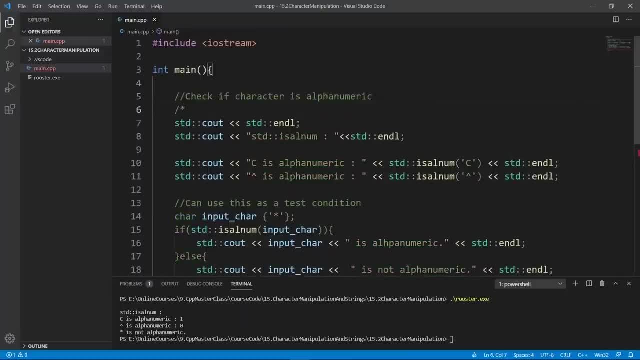 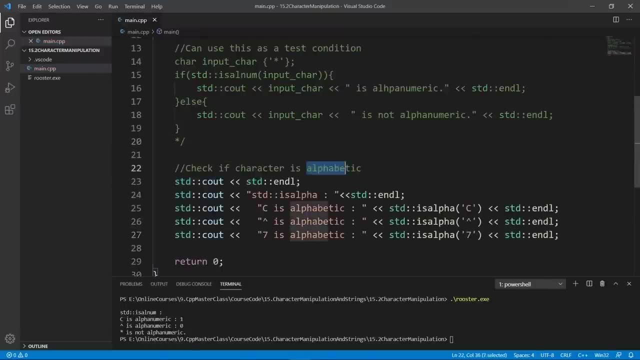 are many of these. we're going to look at quite a few of them. we're going to comment the out and go down and put in a code here and this is going to check if a character is alphabetic. so if it is an alphabet character a from z, lowercase and uppercase c is alphabetic the character here. 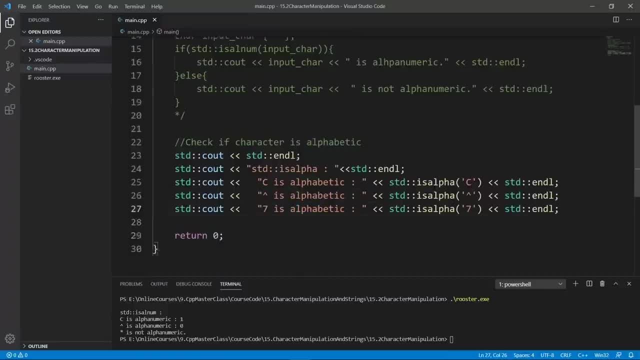 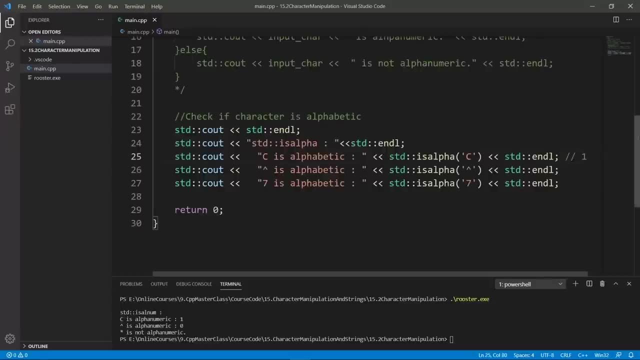 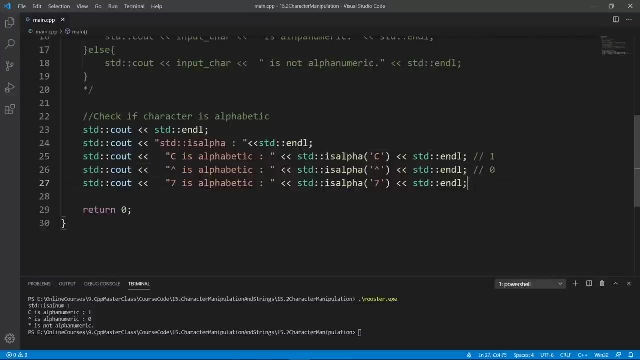 is not alphabetic, and seven here is not alphabetic. so for the first one here, we're going to get something not equal to zero. we should get a one. that's what they use in most cases. for this, we're going to get a zero, a second one, and for the third one, we're going to also get a zero. this is what we. 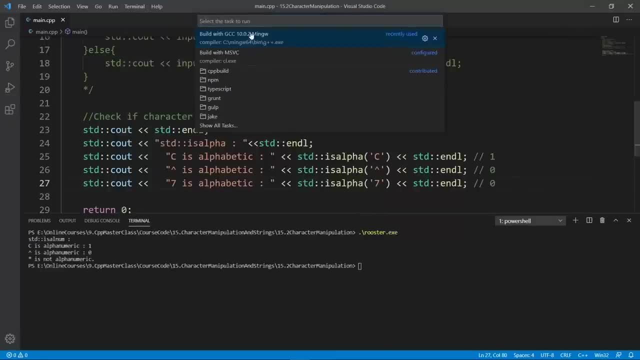 expect. we are going to build with gcc, of course, and we are going to clear and run rooster and we're going to get that c is alphabetic, this guy is not alphabetic and seven is not alphabetic. if we change this c to e, for example, lowercase and build again, you're going to see that the results 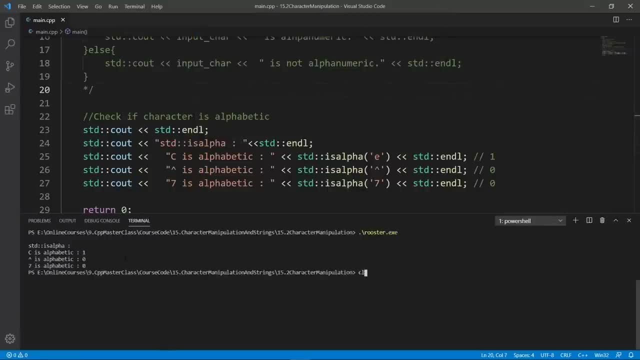 are going to be what we expect. e is alphabetic, that's clear, and run rooster. this is going to be exactly what we expect, but you see that it is not a one and this is not guaranteed to always give you a one. it is guaranteed to give you something. 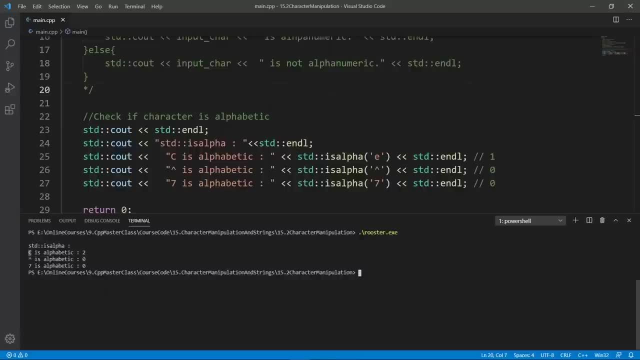 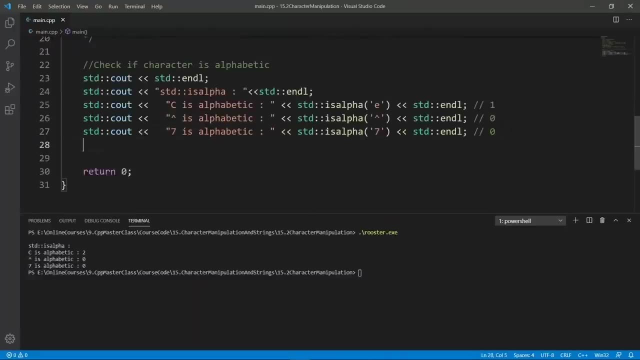 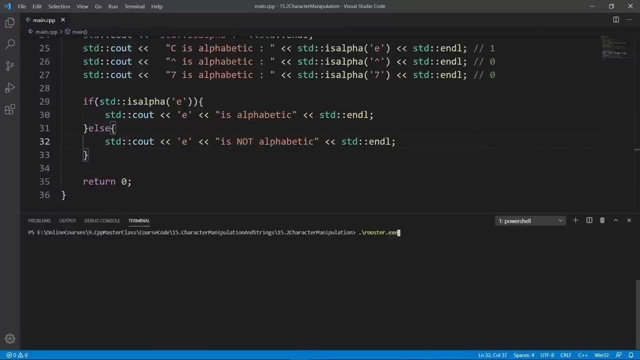 different from zero if the character is alphabetic and zero if not. and we can use this guy here in a test. for example, we can say f, std is alpha, and if we build, the build is going to be good and we're going to get that c and run rooster and you see, e is alphabetic. i should put a space here. i do. 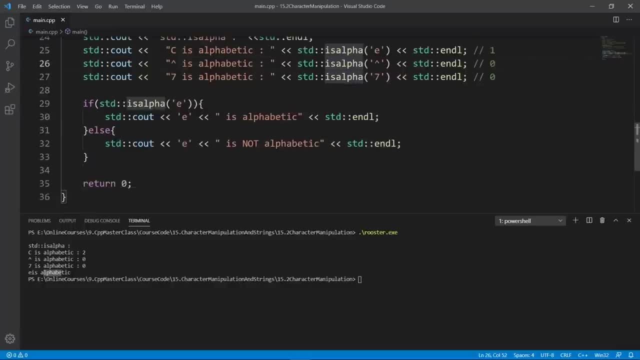 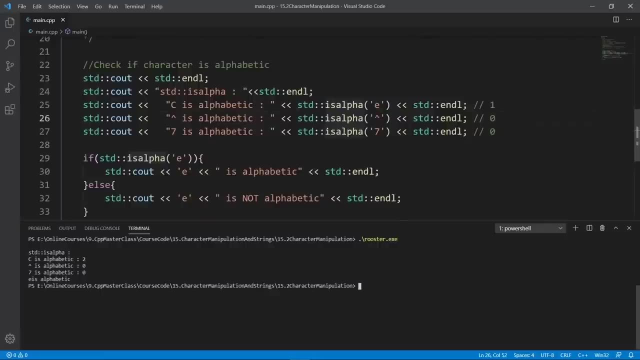 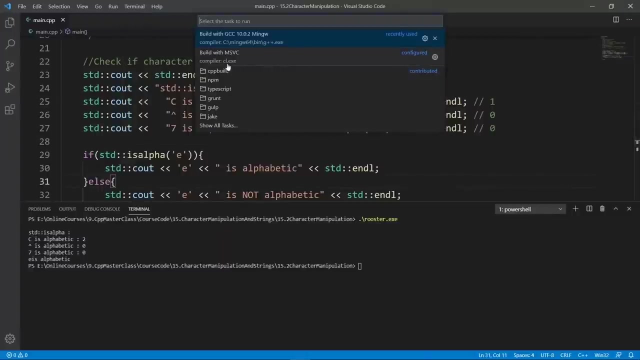 encourage you to change these characters up and see what you get here and see how you can use this things in tests. that's the best way to learn. okay, before we continue, i do encourage you to try and run these methods through different compilers. for example, here we also have an msvc compiler from 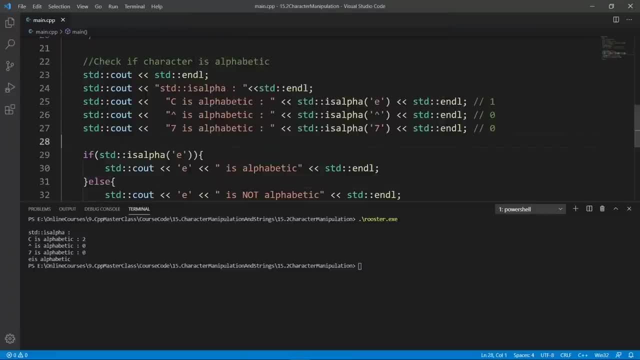 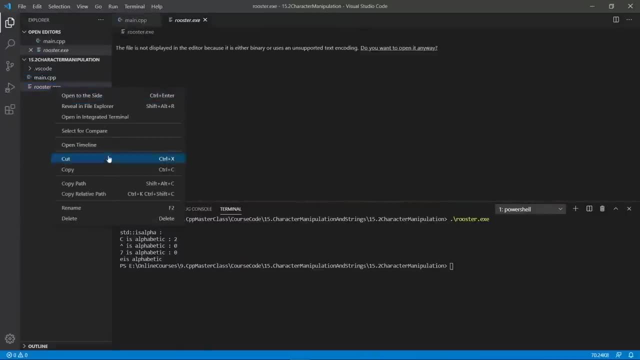 microsoft setup so we can use that and try to build this thing here. but before we do that, let's bring up the c and run rooster and you see e is alphabetic. i should put a space here. i do encourage you to change up our pane here and remove roosterexe here, because we don't want to override it. we're going. 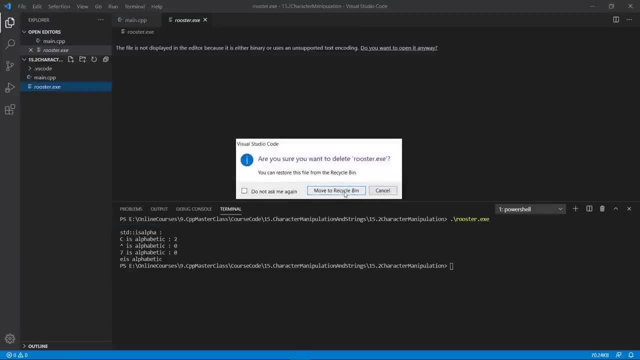 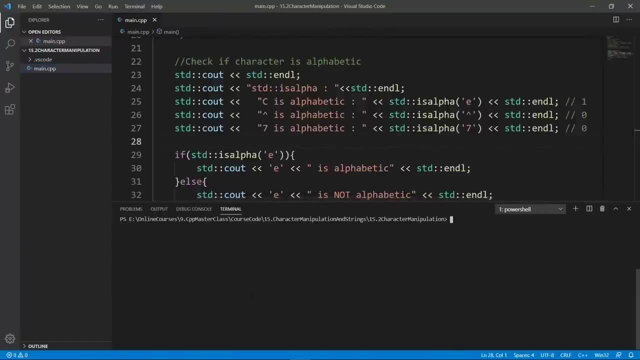 to select it and do delete, and i am going to remove this and move that to the recycle bin and i am going to clear whatever i have here on the terminal and i am going to go there. i'm going to choose run task and i am going to choose world with msvc here i am going to use that. 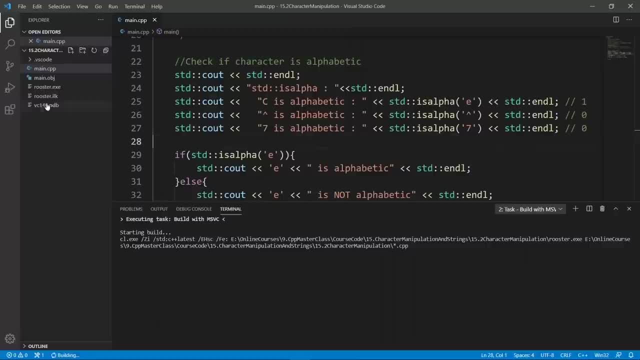 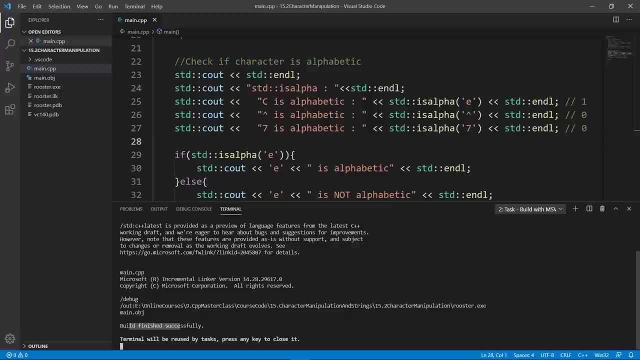 it is going to build my thing. you see the output here and we have roosterexe here and it should say that the world is good in a minute, world finished successfully. microsoft is going to give us a lot of output here, but no problem, the build is good. if we go in, we can actually check. 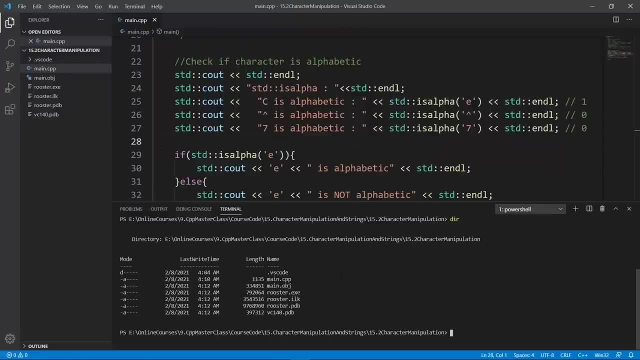 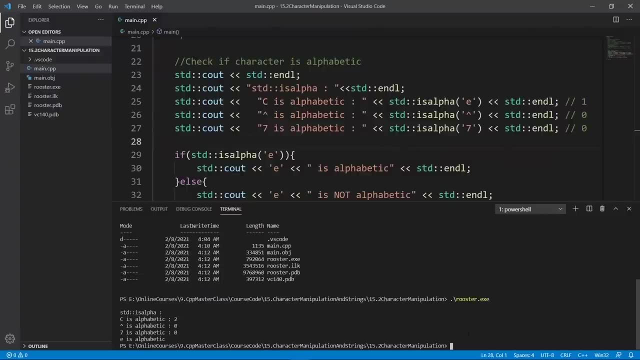 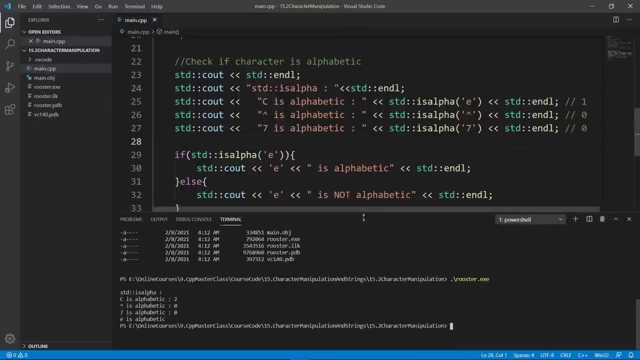 and see what we have in our folder here. you're going to see that we have these files. one of them is roosterexe. if we run it, we're going to see that we have these files and we're going to get the output that we expect. and you see that it is exactly the same thing we got with gcc. i am 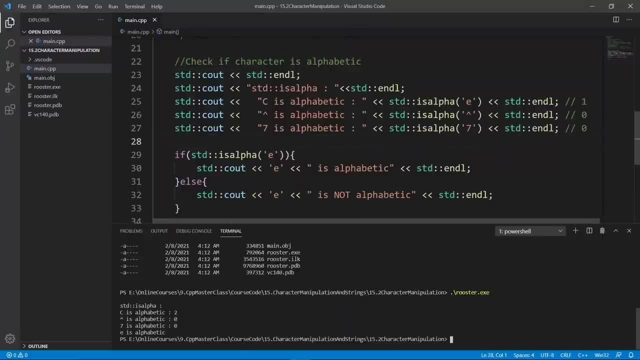 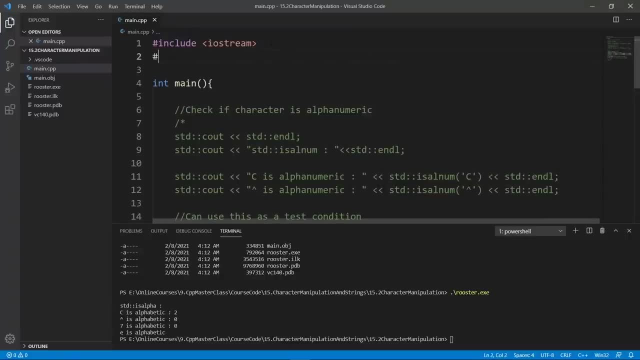 telling you to try and use different compilers, because some compilers are going to flag some of the facilities from cc type, or those that start with c, as unsafe, because there are some things that can really throw you off about them, and we're going to learn about them in this chapter as we 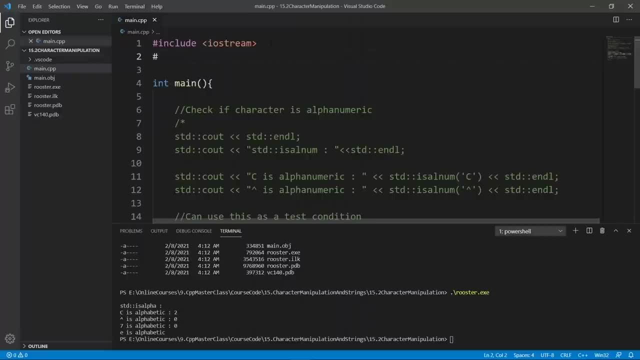 move forward. just know that it is a good idea to try and use different compilers, and we're going to try these things on different compilers and see the errors you get and make yourself familiar with those things. for now we're going to move on and we are going to keep using gcc because that's my 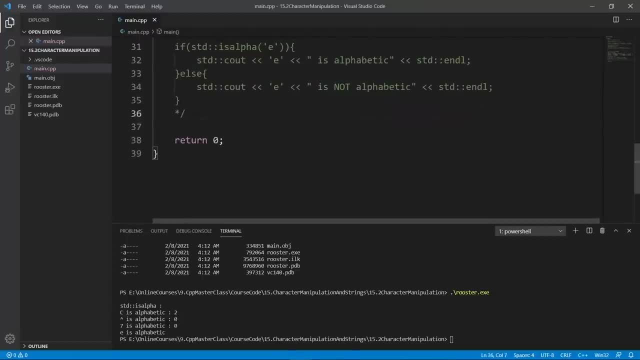 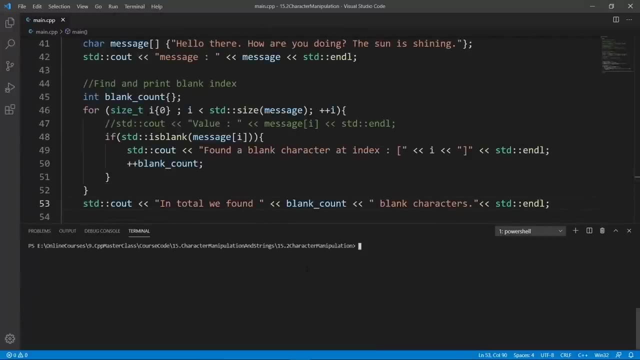 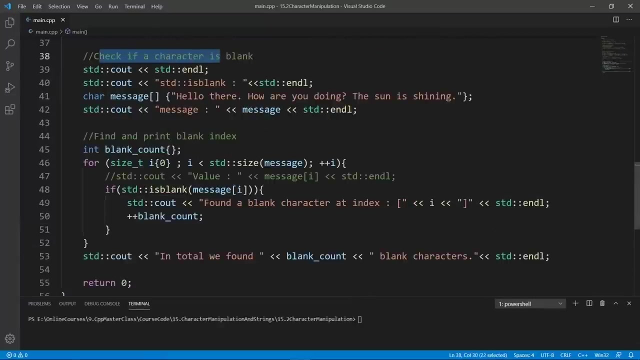 favorite compiler. you can use whatever compiler you want. the next example is going to check if a character is blank. let's close this thing and clear and give ourselves some breathing room. we're going to bring this down a little bit and we're going to check if a character is blank. the 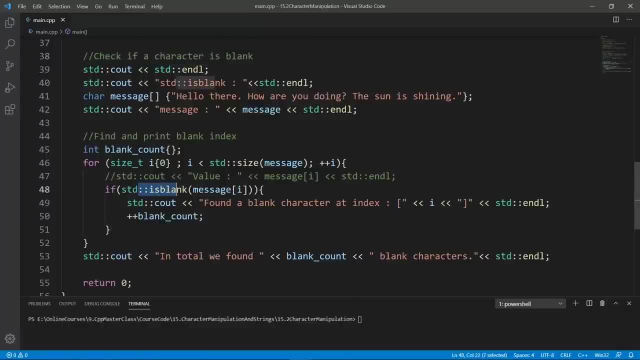 reality, for that is, std is blank, and if it's a blank character, we're going to get something different than zero and we can use that in a test like this. and if it's not a blank, we're going to get something equal to zero and this test here is going to fail. so what this example here is going? 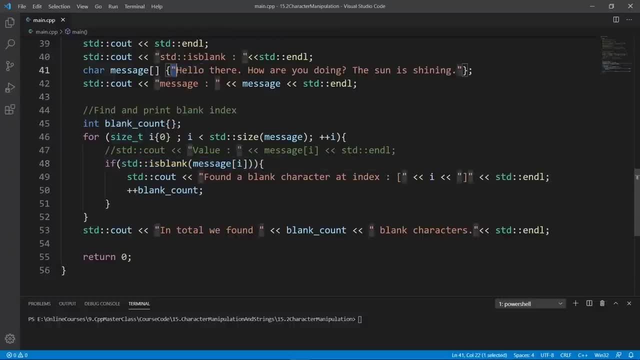 to do. it's going to count how many blank characters we have in this message here, and we're going to print the counter of that on the console using this line here. so let's go through this loop and see what it does. the first thing we do is initialize. 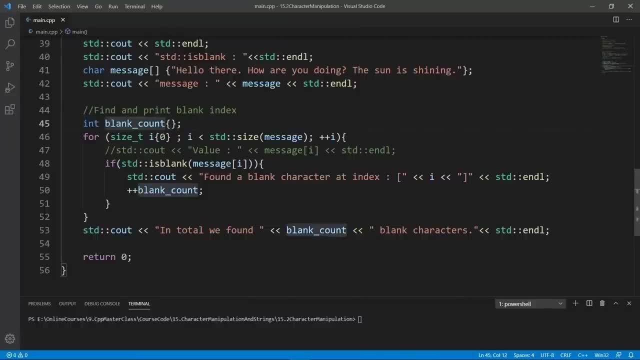 blank count to zero and we are using an integer. and because this is a count, i think blank count is of wrong type because it can be negative. so to really be safe in our program here, we should make this unsigned or even use size t. this is better, okay. so let's use size t, because this is a size. 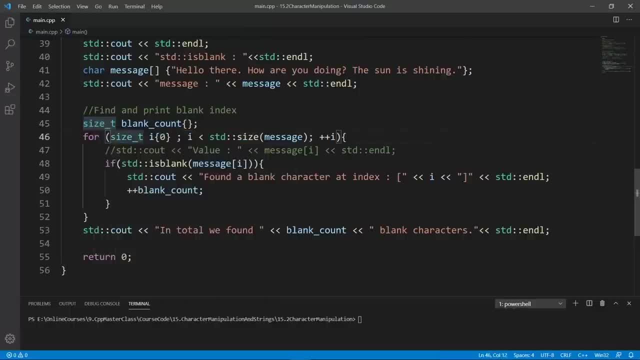 and size t is a good type to keep track of sizes in your c++ programs. so make sure you use size t here. and what we're going to do is go in the loop at each iteration. we're going to check if each character at each iteration is a blank. if it is, we're going to fall in here and say that we found. 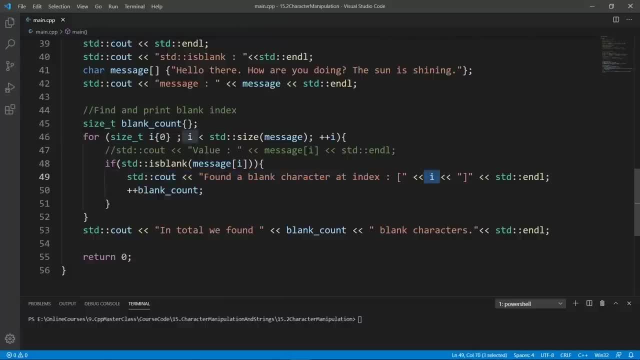 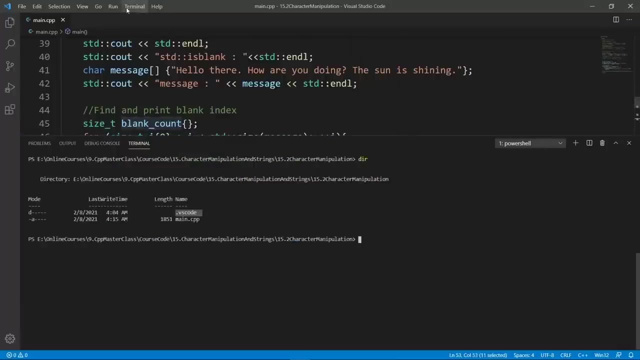 a blank character at this index in our array here and we're going to increment our blank count and by the time this loop is done, we're going to have the blank count stored in this blank count variable and we're going to print that out. it is this simple. now we can build with gcc. 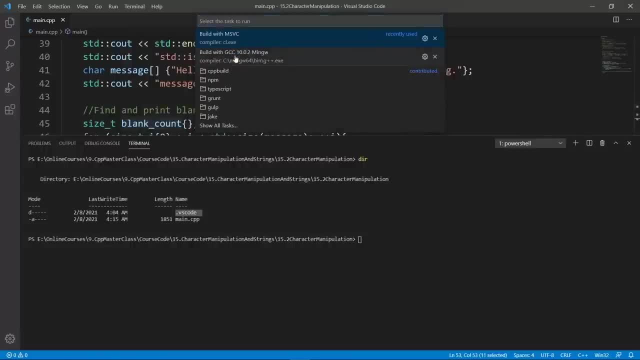 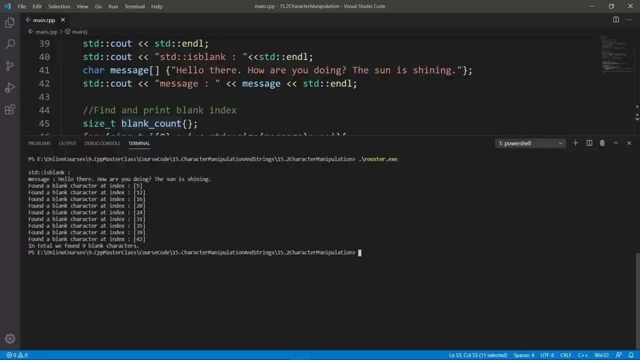 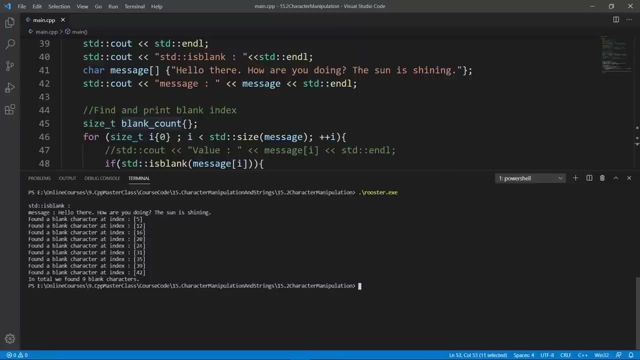 let's do that. we're going to world with our gcc compiler and the world is going to be good. we can clear and run rooster and you're going to see that it's going to say: we found a blank character at index 5, 12, 20, 24, 31, 35, 39 and 42 and in total we have found nine blank characters. 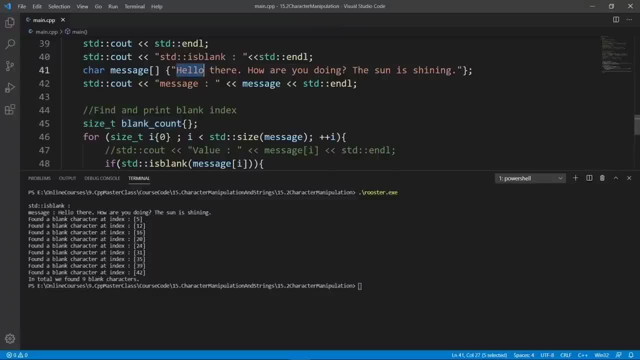 do we have that many? let's count. so one, one blank character. we have two, here we have three, we have four, we have five, here we have six, seven, eight and nine. if you count you're going to find that we have them and the first one is at index: five, so index. 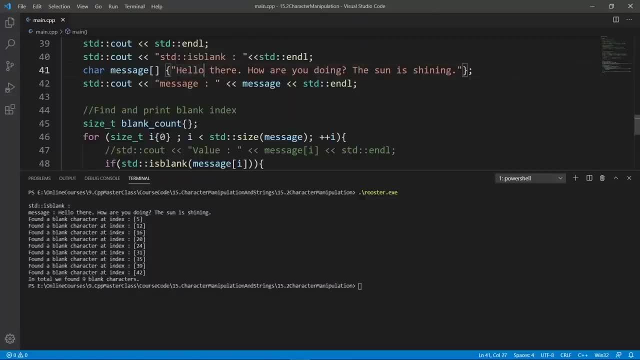 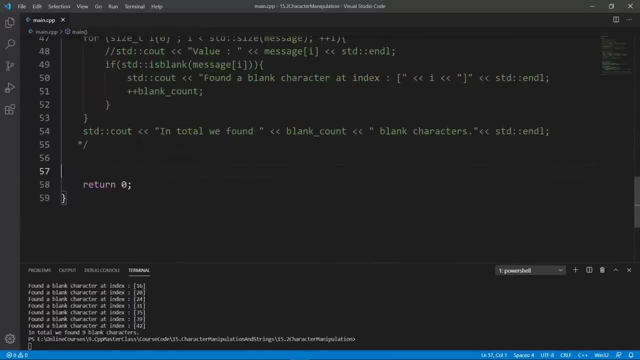 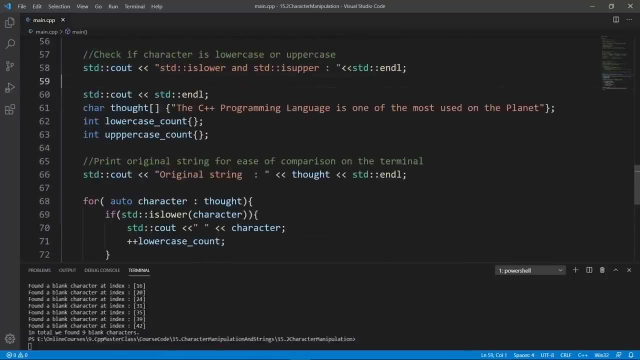 zero is h. one, two, three, four. the first one is at index five, and this is doing exactly what we want. we can go down and check if a character is uppercase or lowercase. we can do that through an example like this, and the facility is going to be std lower and std is upper. we have a message. 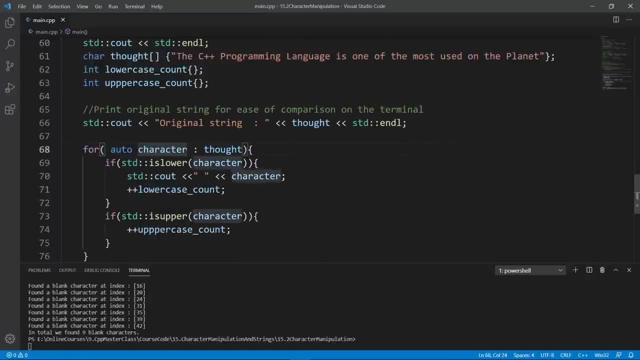 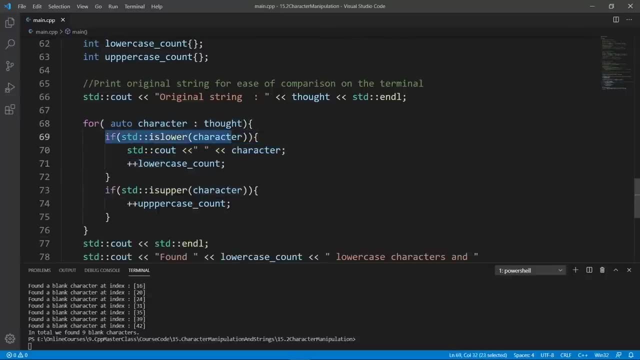 here we're going to loop around using a range based for a loop and we're going to check if each character is either lowercase or uppercase and if the test is good, we're going to jump in the loop and we're going to increment lowercase count, which are a few variables to keep track. 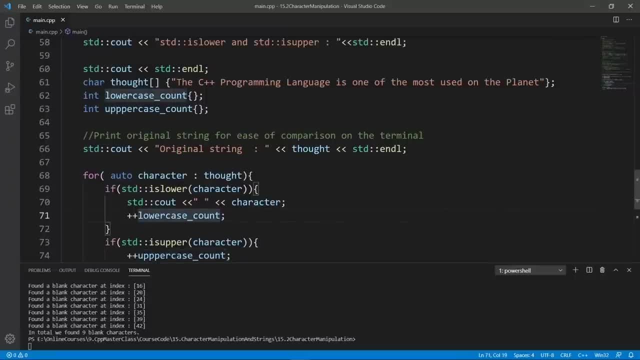 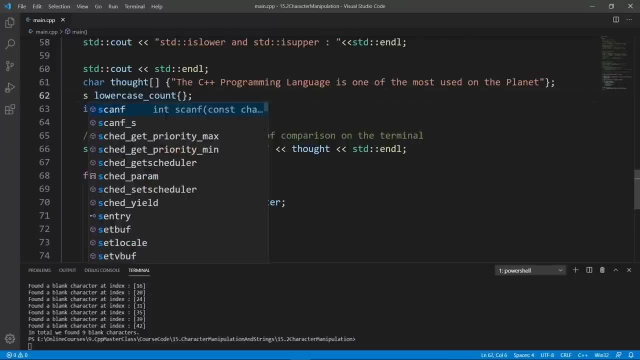 of how many uppercase and lowercase characters we have in here and again these variables are going to count. so it is better to use size T or some unsigned integer type. but now we're going to use size t because it is good. so we're going to keep this stored in here and we're going to build this. 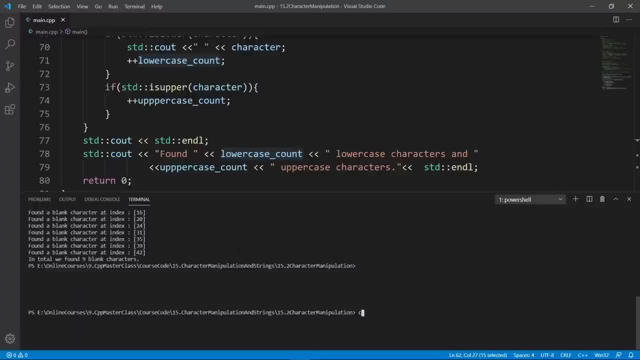 and see what we get before we run. we want to clear and we are going to build with gcc. the build is going to be good. we're going to clear and run rooster and you see that the original strand is this guy here. what we're going. 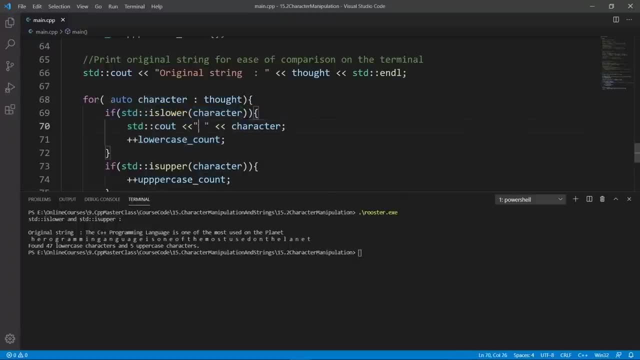 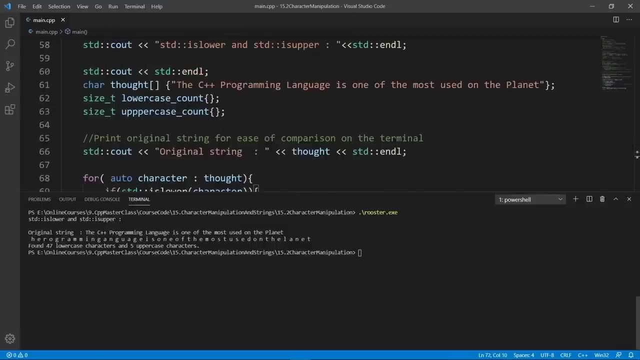 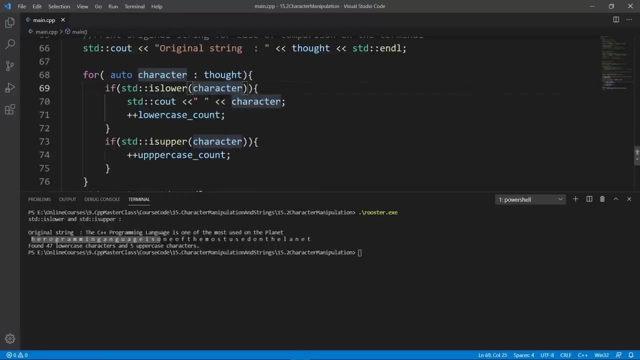 do? we're going to print whatever character we are at, we're going to put a space in front of that and we're going to see increment. this is the output. why do we have this message here? because we are printing out each character and we are not printing the uppercase ones. we are printing lowercase ones. 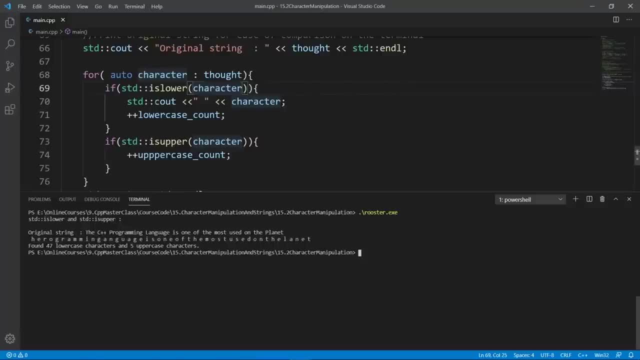 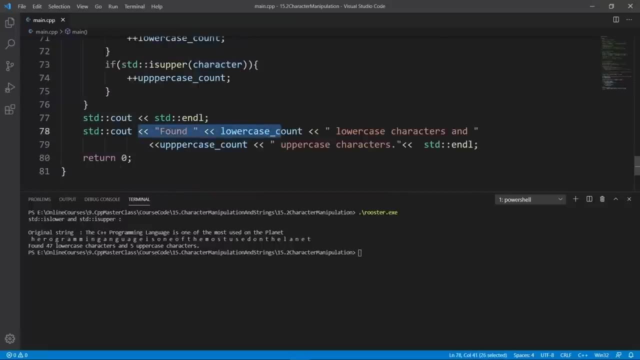 that's why you see this guy here. this is really interesting. you can keep this in if you want. i am going to keep this on. the important message is that we found lowercase characters and uppercase characters and we have five uppercase characters. if we go in and count, we're going to. 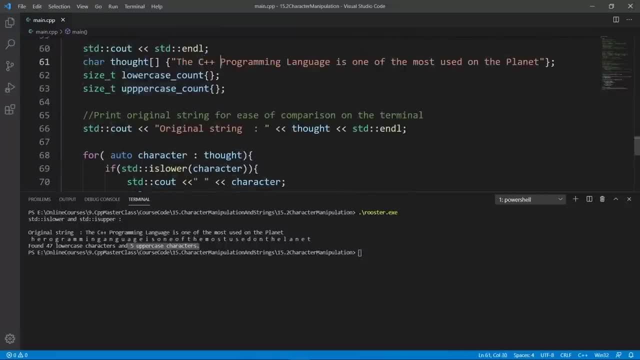 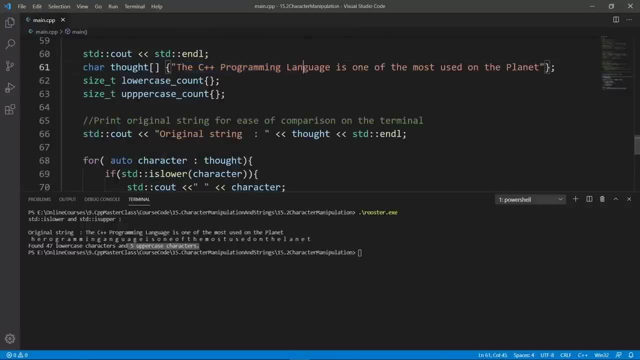 find that we have t here, one, two and three and four and five, five uppercase characters, and if you count the lowercase characters one by one, i am sure that you're going to get a 47, like we did here. we're going to comment this out because this was just an example. 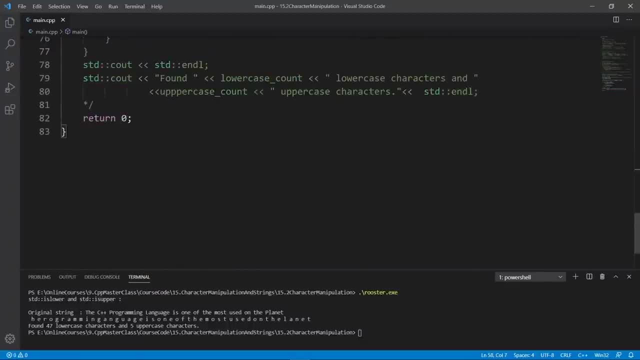 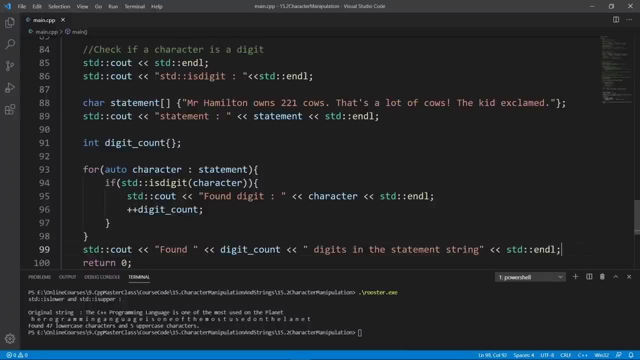 i am leaving this in here so that you can use this as a reference if you want. we can also check if a character is a digit and we're going to use std is digit to check that the return type is going to be different from zero if the test succeeds. if it fails, we're going to get a zero. 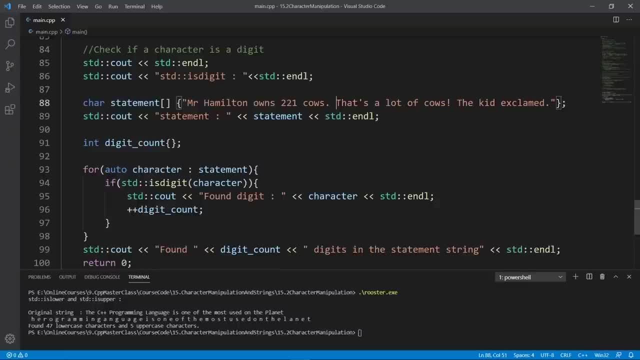 and we can use that like this. so we have a message here stored in the character array called statement, and we're going to loop around checking if each character we are at is actually a digit or not. if it's a digit, we're going to say: found a digit. i'm going to say: 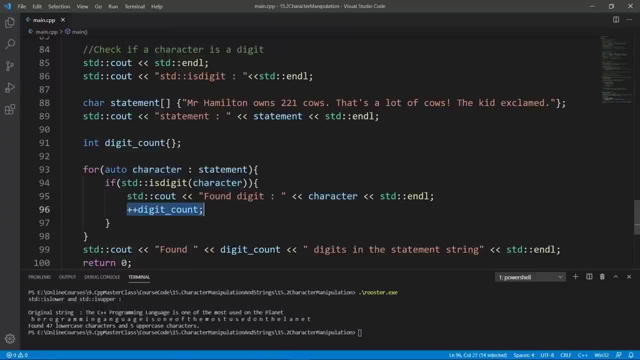 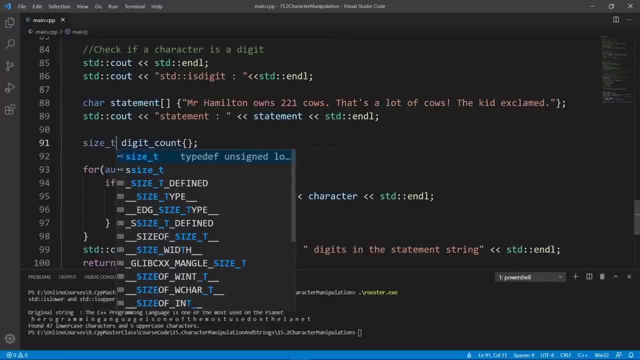 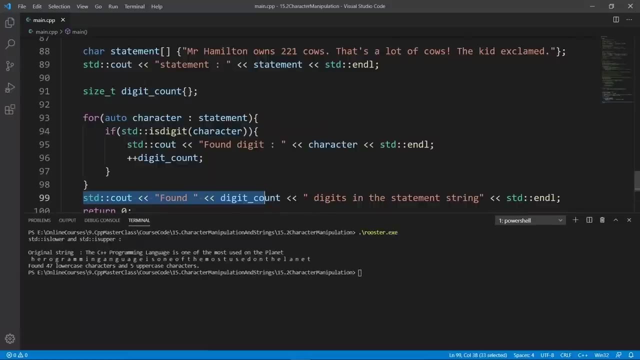 whatever digit we found and we're going to increment the digits count and we're going to store that information in this digit count variable. here we don't want to make it an end, so we're going to make it a size t and we're going to build and run this program and see how many digits. 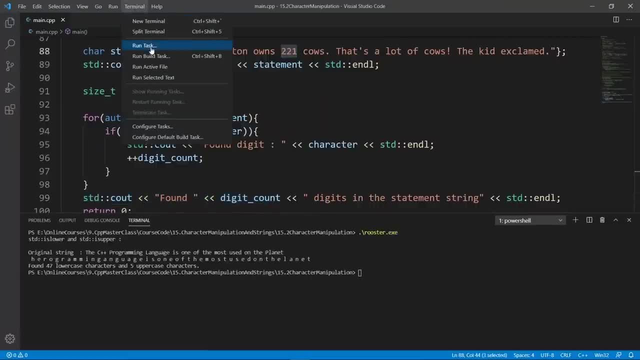 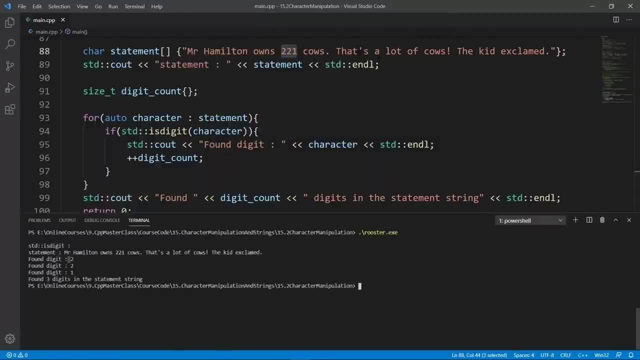 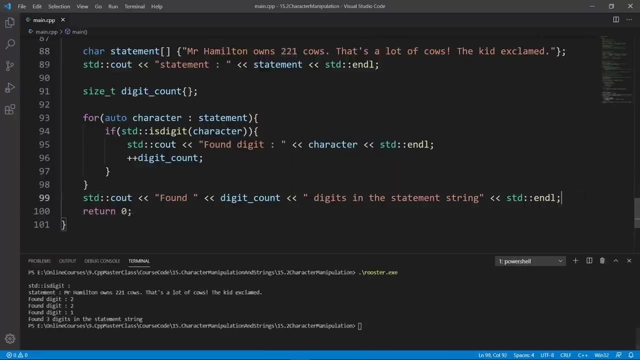 we found- you know it is this number here, i'm not going to say it, we're going to let our program figure this out. so, rooster and we're going to find two, two and one. so we found three digits, and it is exactly what we expect here. we're going to comment this out and show you another example. 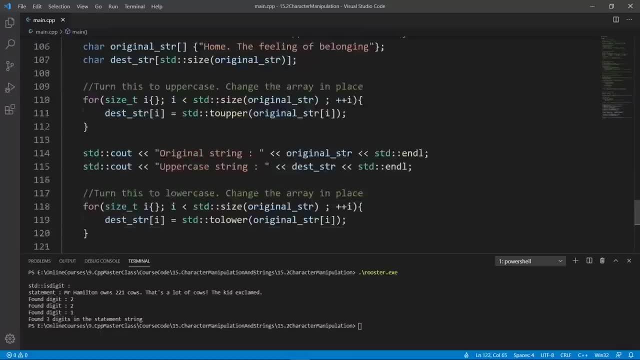 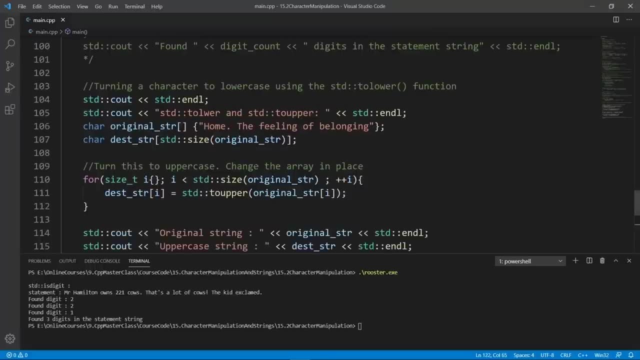 and in the last example we're going to be showing you that you can change the case of a character: if it's lowercase, make it uppercase, if it's uppercase, make it lowercase, and you can do things like that. we have a message here stored in our character array, called original. 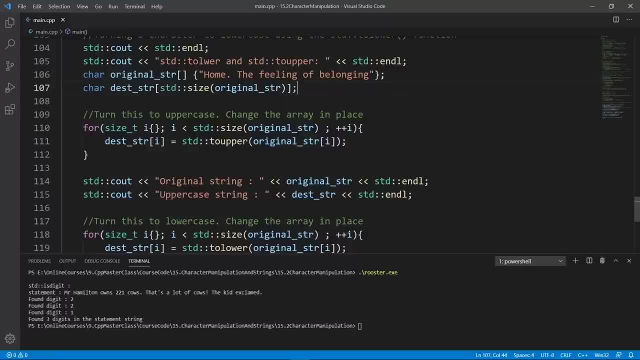 dot inner and liftr, we set up another array which is going to store our message that is transformed and we're going to look around turning everything we come across uppercase the way we do that, we're going to say std to upper and we're going to pass in the character that we want to turn to. 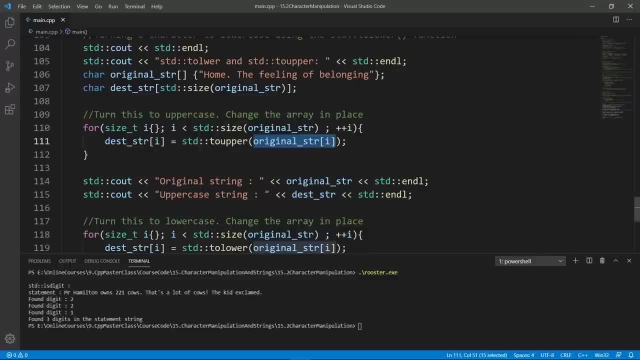 uppercase. if we do that, we're going to get an uppercase character out of that and we're going to store that in our destination array at this index. here it is this simple that we're going to print the original string and the uppercase string. we should get that printed. 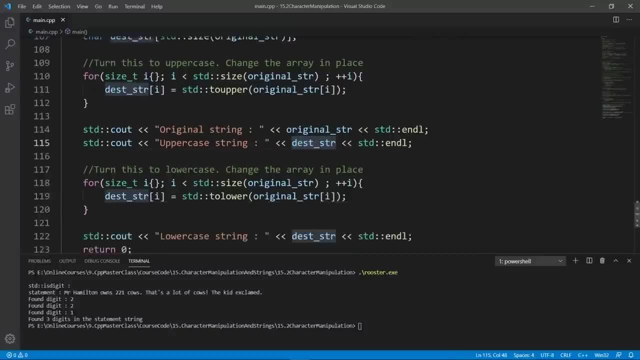 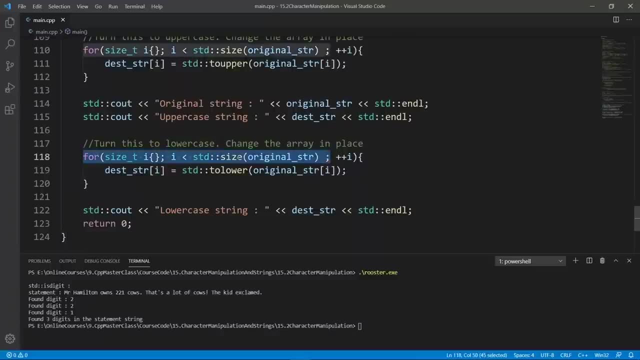 out because it is stored in destination string here and we're going to do the reverse and turn that back into lowercase. we're going to grab the original string, loop over it and at each iteration we're going to get whatever we have and turn that to uppercase, to lowercase, i should say. 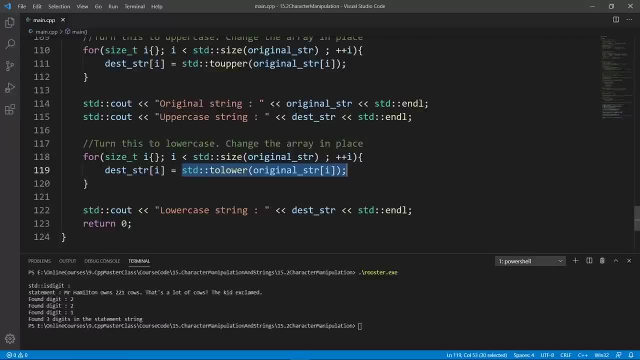 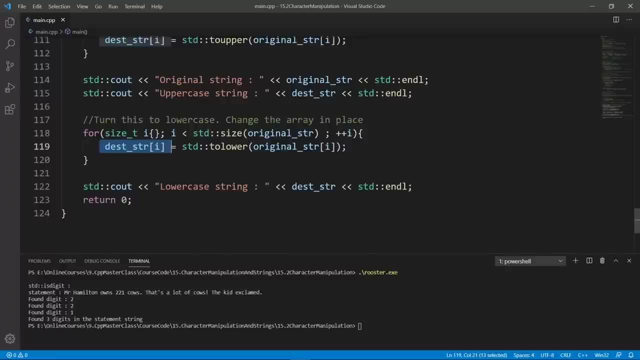 and the result of that is going to be stored back in our destination of strength. so we're going to overwrite whatever we have in our destination string here and after that we're going to print the lowercase string and we should get that printed out. this is how the example works. 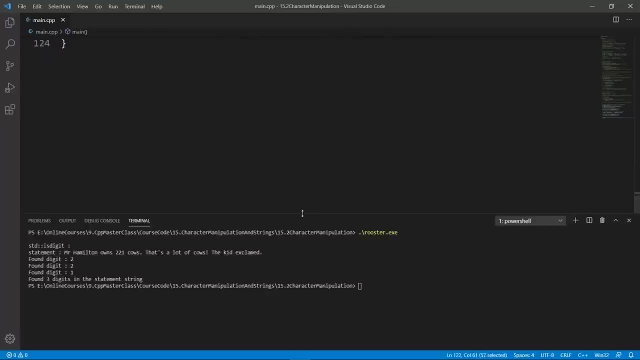 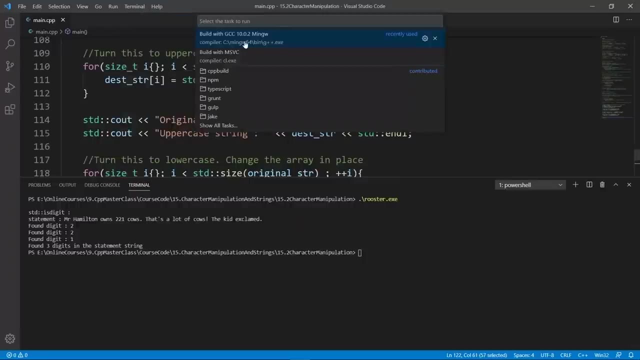 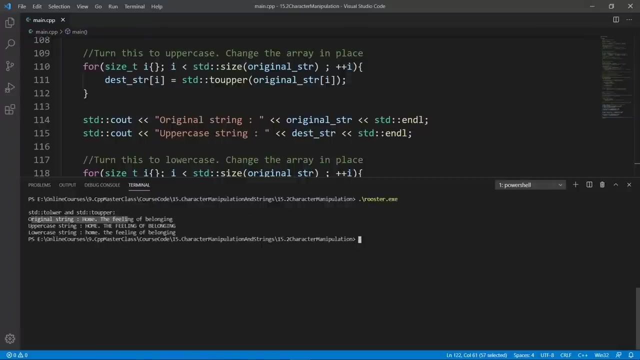 and if you have any problem understanding this- i am always around. please do ask. i will do the best i can to help you out. for now, we are going to build this with gcc. the world is going to be good, we're going to clear and we're going to run rooster and we're going to see that the message 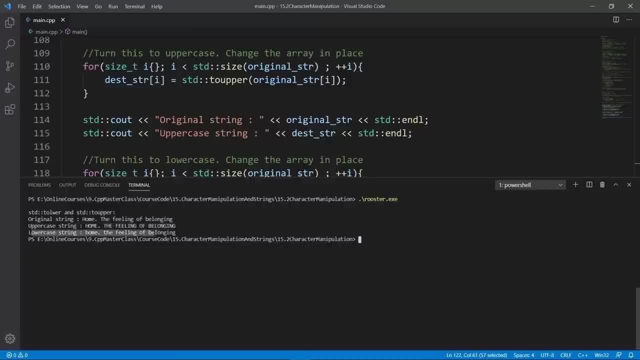 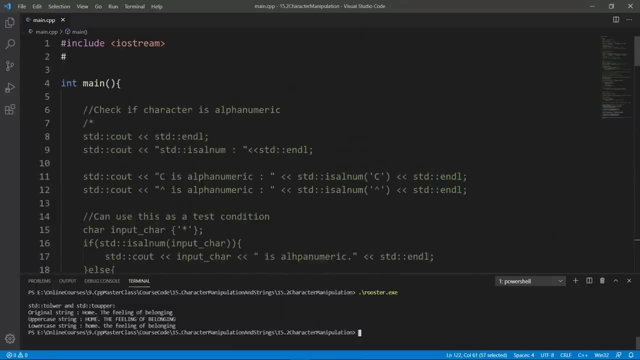 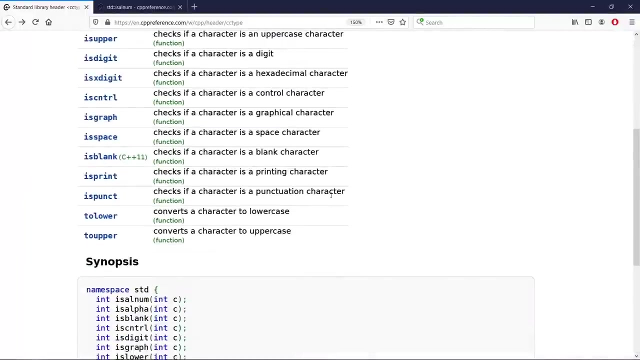 is here. it is turned uppercase, it is turned lowercase, and this is how you can do these things here. so we have looked at a few of these facilities from cc type. i don't really want to look at all of them because that would be really boring. i hope you have an idea about how they work. 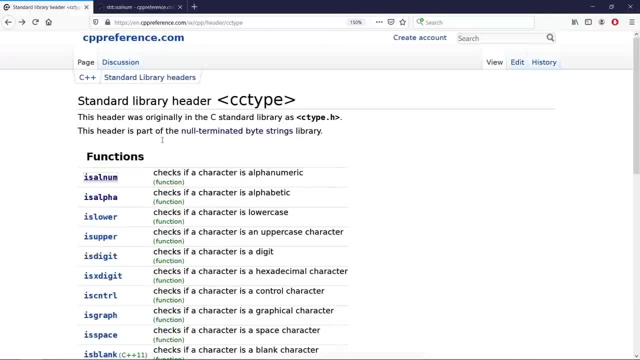 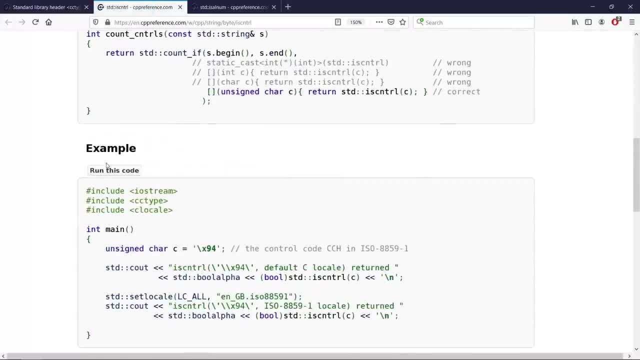 and if you want to look at all of them, all you have to do is come to the documentation here, choose one, open it up and look at the documentation, and in most cases they are going to have examples down here that you can look at and play with. for now, we are going to stop here in. 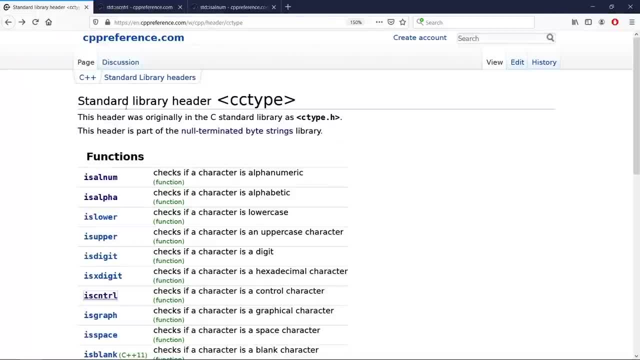 this lecture. this is really all we set out to do to play with many of these facilities from the cc type library. in the next lecture we're going to look at how we can manipulate c strings, and by that we mean concatenating them or putting them together, copying them out and doing all kinds of 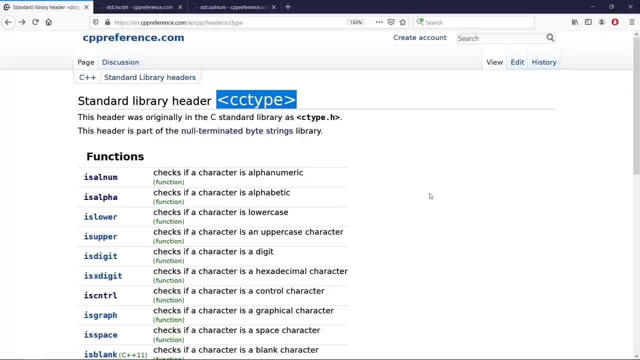 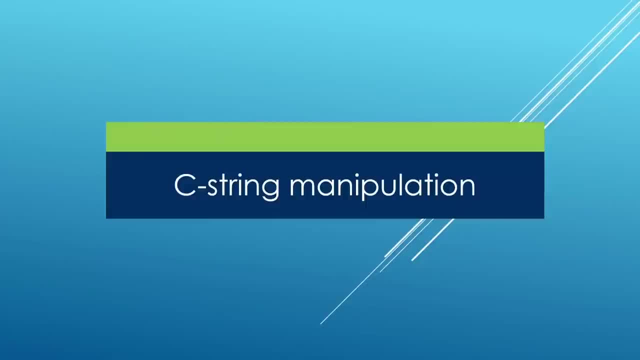 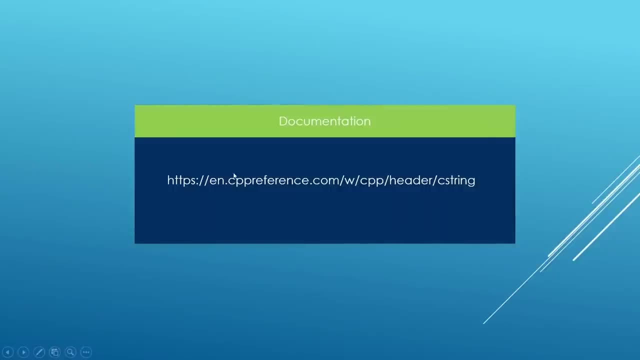 crazy things go ahead and finish up here and meet me there. in this lecture we're going to look at the facilities from the c++ standard library to play with c strings. all of these are going to be leaving in the c string library- you can go and check it out at cpp reference- and we're going to start. 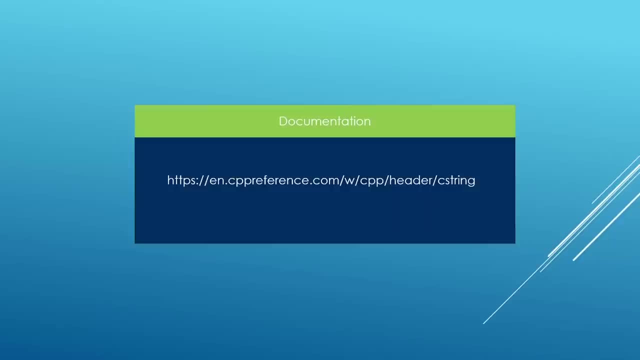 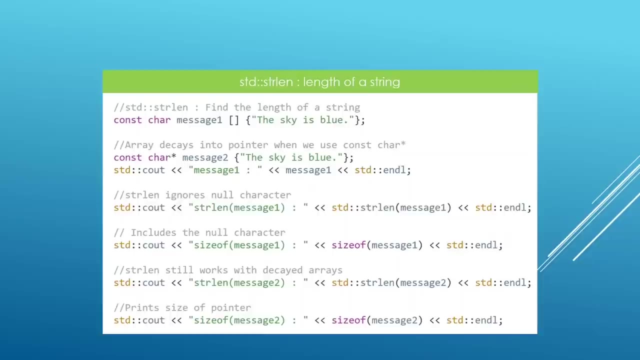 and look at a few examples of some of the things we can do with this library. i mean c string. the first thing we're going to look at is an example of how we can check the length of a string. here we have a character array called message one. it is a character array and you see that we made 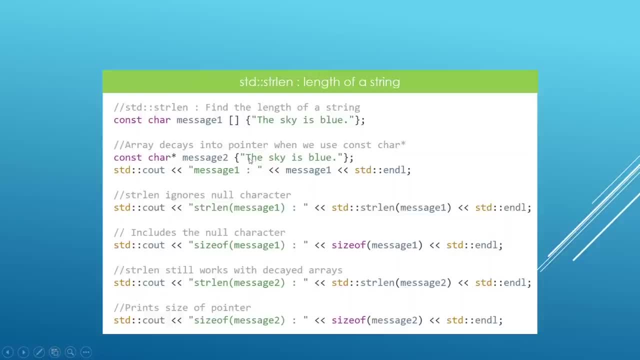 it const. we also have another array that is pointed to by pointer. you know that if we do things like this, this array is going to decay into a pointer and there are a few things we can do with it. for example, we can't use it with std size and we can't use a range based for loop to loop through this. 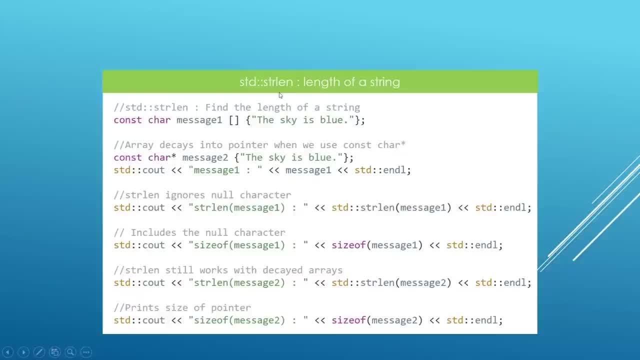 message to thank you, but str length is going to decay into a pointer and we can't use it with std. then it's going to help us check the length of this thing here, so we can use it. for example, if we do std, strlam message one, we're going to get the number of characters in this string here. this is: 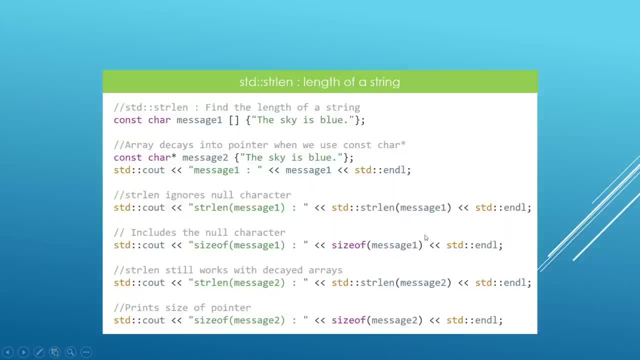 not going to count the null character, though, so the null character that is implicitly added in by the compiler is not going to be counted in here. you're going to see this in a minute when we hit visual studio code to play with this. thanks, but this facility can work regardless of the. 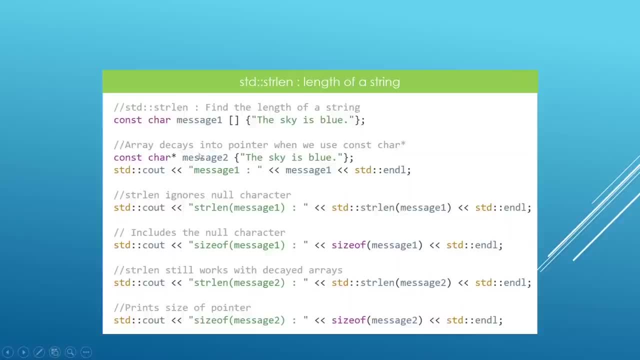 number of characters in this array. so it's going to work regardless of whether you are using a row array like this or even for pointers like this, and it is really cool, so we can use it like this. we're going to get it printed out. please know that we can also use the size of operator to get the same. 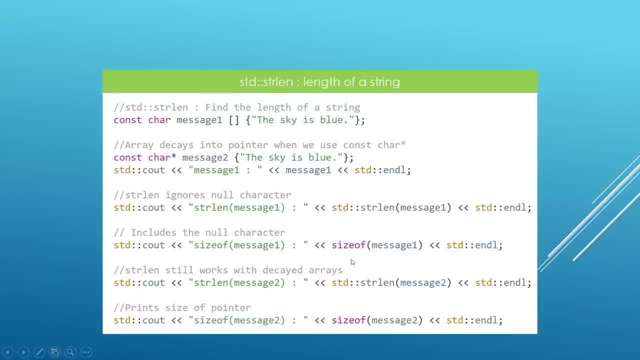 thing. so it is going to work almost the same way, but the size of operator is going to include the null character. you need to be aware of this. the good thing about str len here is that it still works for a decayed arrays, so if we use it, 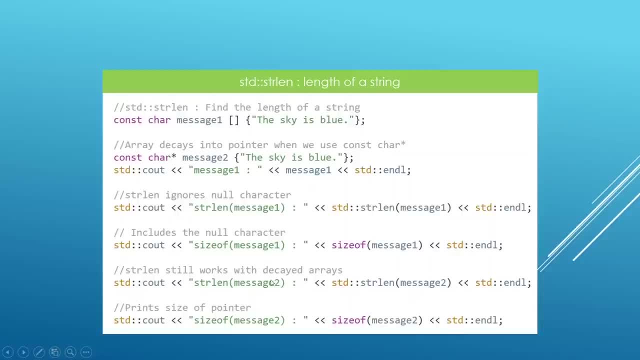 on message 2. we're going to get the correct output. we're going to get the number of characters in here, which is really cool, and we can also try and print out the size of message 2, but here we're going to get the size of a pointer printed out. okay, that's how str len works. it lets you evaluate. 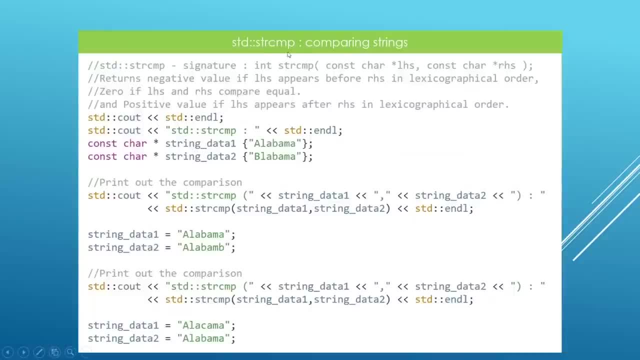 the length of a string. here is another example, and it is str, cmp or string compare. it is used to compare strengths. what you're going to do with this facility is give it two strands- c strands, we should be exact- and one is this guy here, lh ace or left hand. 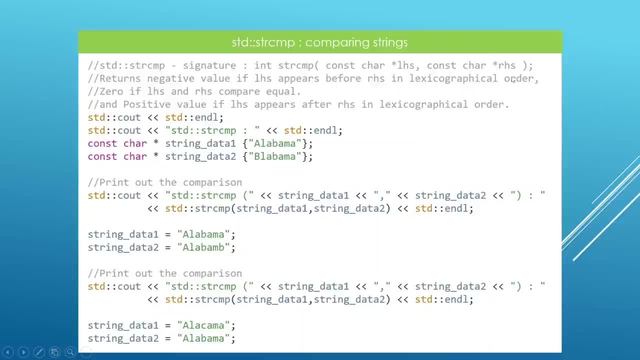 string. i think that's what this stands for and we're going to give it a right hand strand. and, by the way, these signatures are copied straight from the documentation so that we can look at this in one slide to make it really easy to follow. this is going to return a negative value if 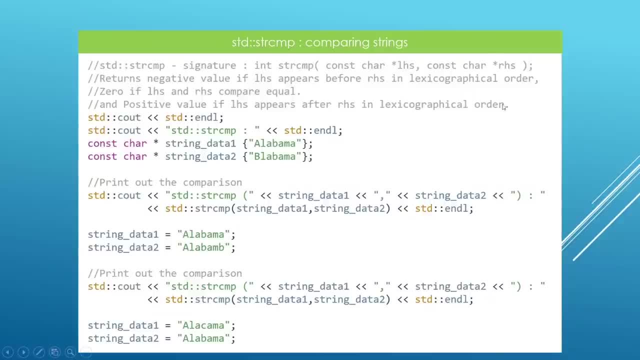 the first guy happens to come before the second guy in lexicon co-graphical order, so it is something like a comes in front of b, c comes in front of d or something like that. if the two strengths are equal, it is going to return zero and it's going to. 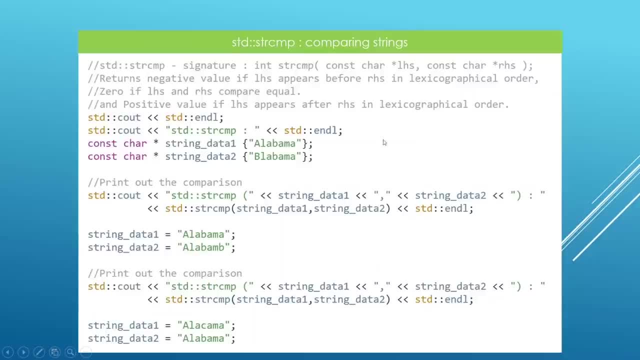 return a positive value if the first guy appears after the second guy. okay, and we're going to try it out. we have two strengths- alabama and blabama- here, and they are stored in character arrays that are pointed to by these two pointers- string data one and string data two- and we can do something. 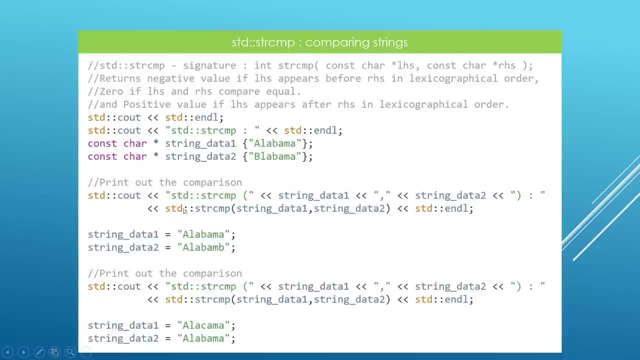 like this below here: so we're going to print something out and we're going to say std, string compare and we're going to pass in the first string and the second string. for now i want you to pause a little bit and try to guess what we're going to get printed out here. the first trend is: 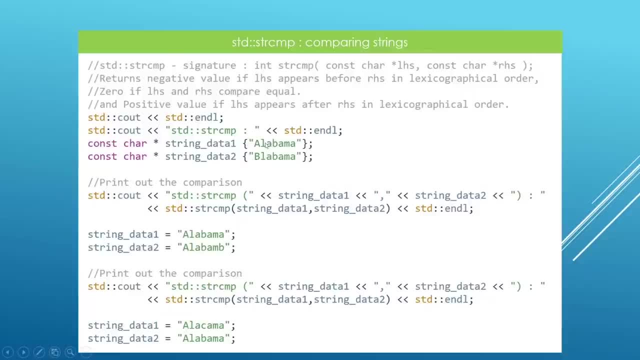 alabama, the second one is blabama, so the first one comes in front of the second and we see that we're going to get a negative value if the first guy comes in front of the second guy. so alabama comes in front of blabama and we would expect to get something negative from this thing we are doing. 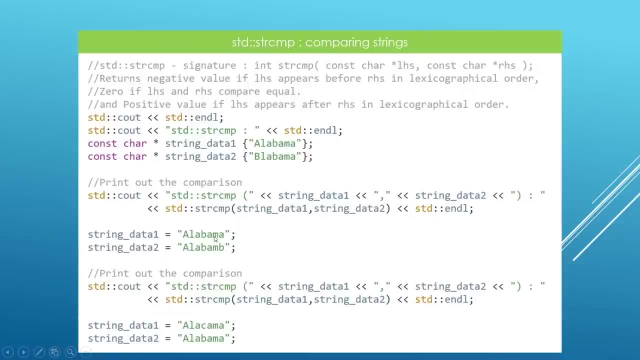 here and again. if we try and change the map a little bit, you see that alabama still comes before alabam. so we're going to get a negative value pointed out and we can change these things up to see what we get. it is really simple. if you know how to use them, we can also use another. 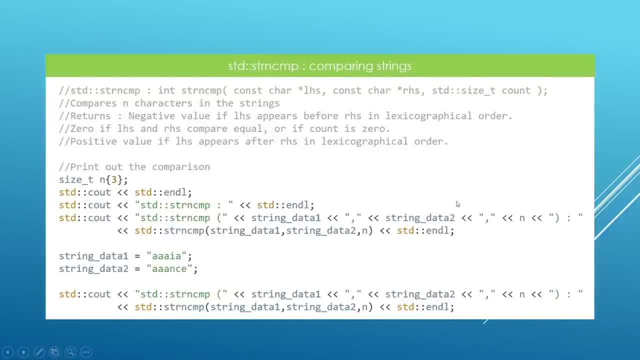 version of string compare, which is going to let us specify the number of characters that we want to compare and specify that we want to compare any characters. in this case it is three characters and it is going to compare a section of the strings that you specify as a first and second parameter here. 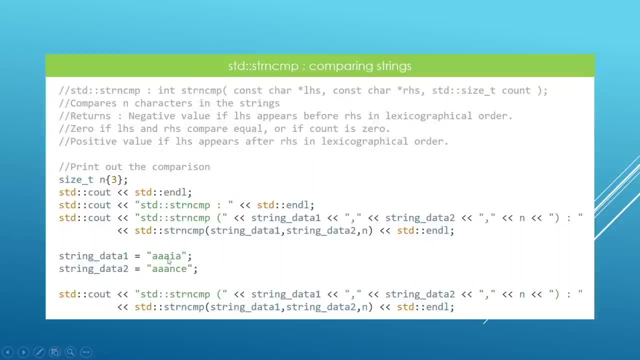 so, for example, if we change string data 1 to be a, a, a, i, a and string data 2 to b, a, a, a, n, c, a, and we are comparing the three characters in here. so we are comparing a, a, a to a, a, we're going to 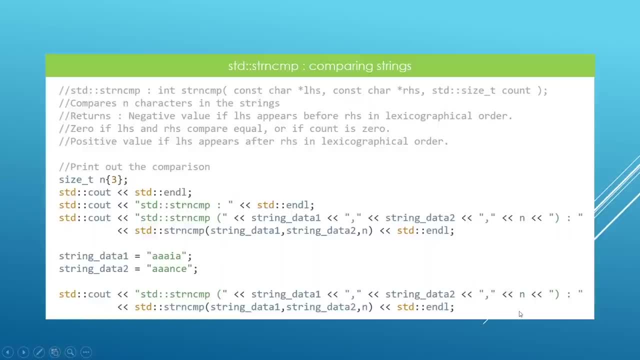 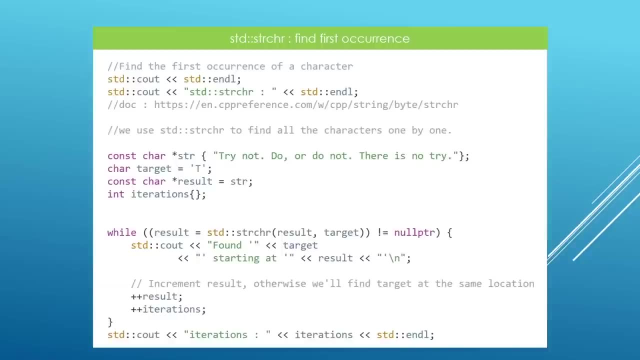 see that they are equal and we're going to get a zero printed out here. you're going to see that this is exactly the case when we get to play with us in visual studio code in a minute. we have a facility that we can use to search in a string and search for a character: the facility for. 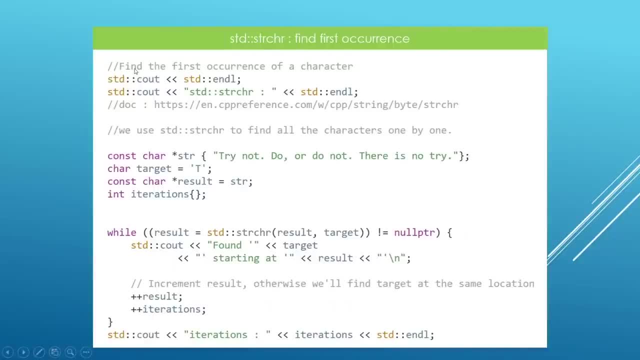 that is str, chr, and it is going to find the first occurrence of a character in a string and the documentation for this is right here, and please note that this example is actually copied straight from the documentation. okay, so we have a message here. it is a character array and it is pointed to by a const car pointer called str, and we have 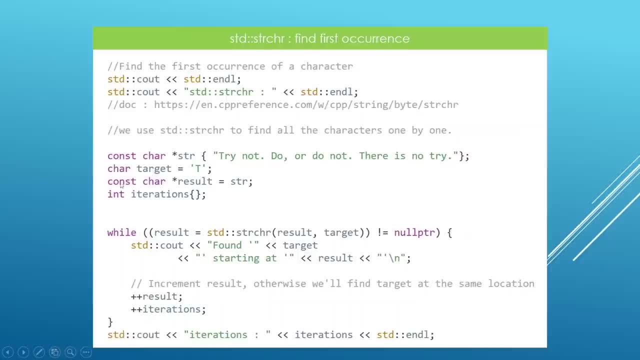 a target character that we are looking for and the result is going to be stored in the reserved character array here and we have a variable called iterations that is going to keep track of how many iterations we did to find our target here. the way this guy works. 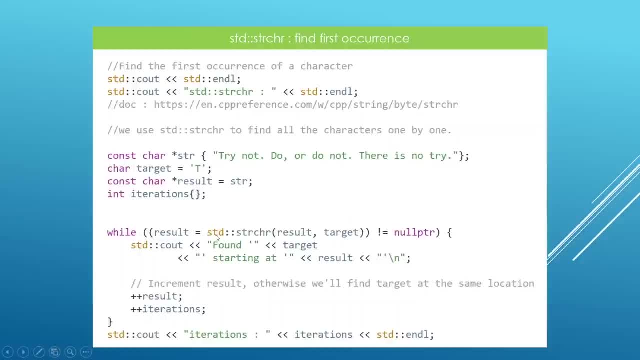 it is going to return a pointer to what you find. if it is found, for example, in here, if we find this first t, this function here or this facility is going to return a pointer to this first t here. if it doesn't find what we want, it is going to return a null pointer. that's how it. 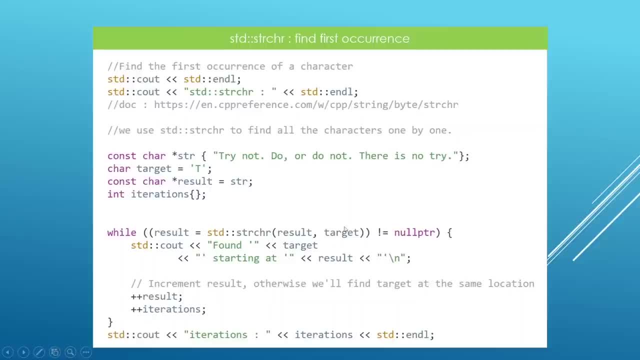 works and you can see that in the documentation here we are going to take advantage of how it works in this while loop here and the way you use this facility. you give it the strength you want to search in and you give it the character that you are looking for. so if we look at how it works in 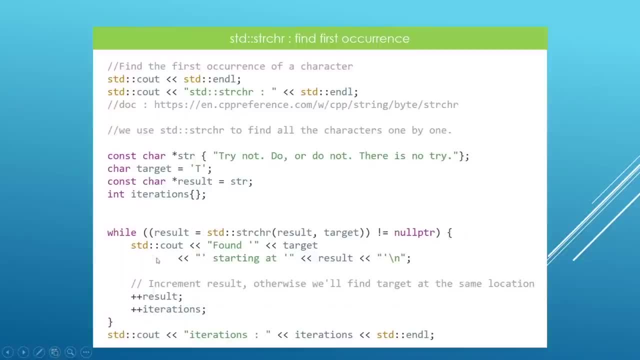 we are going to call the function and we are going to store the result in our character pointer here and if we go inside we're going to hit the first character here at the first iteration. so we're going to find this t here and when we find it, the result of this is going to be: 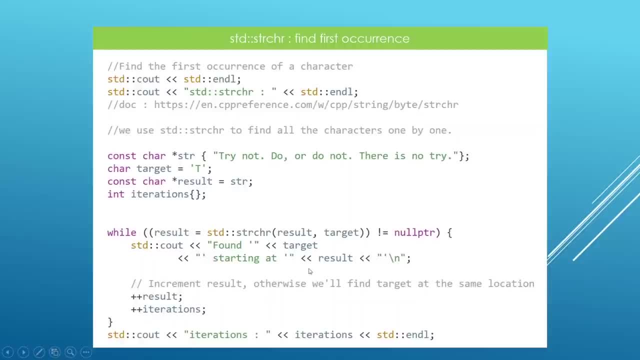 stored back in reserve here. i hope this makes sense. so we're going to find it, we're going to print it and we're going to increment reserve. to make it point to the next character, this is pointer arithmetic in action here and after we do that, we're going to increment the iterations, so we should have one iteration by now. 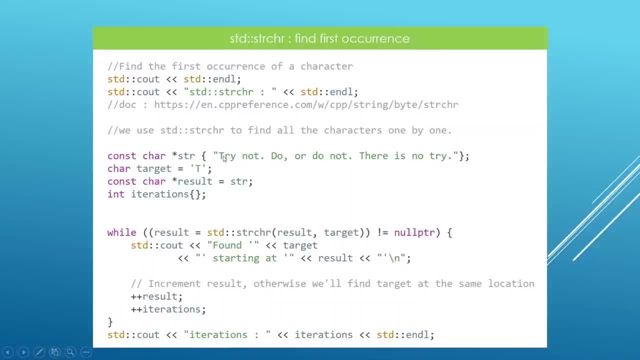 and we're going to jump into the loop again. so the string we search in is going to be starting from r here. so we're going to try and find an uppercase tn and it is going to find this uppercase t here. so it is going to point to it and the pointer to this t is going to be stored. 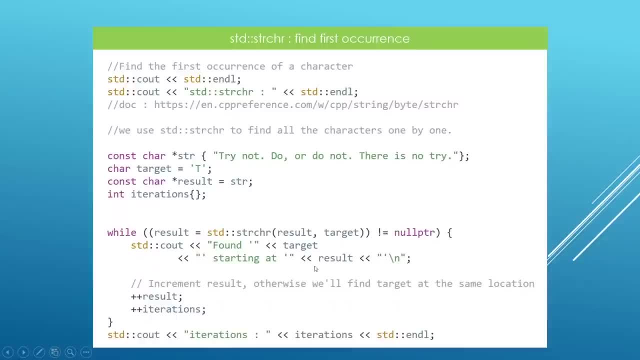 in this result here, okay, and we're going to jump into our body here we're going to say that we found this t, we're going to print it out and we're going to increment reserve. if we increment reserve now, reserve is going to be pointing to the h here, okay, and we're going to say how many. 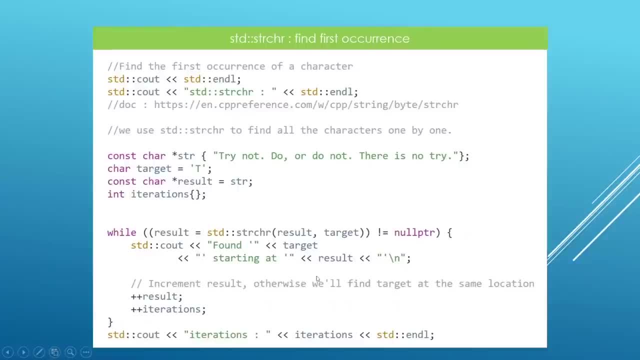 iterations we did to find our thing. we will have printed out the t that we have found and we're going to jump to the next iteration, which is going to be searching for t in the reminder of the string here. it's not going to find it, of course. it's going to return no pointer. and the test here is: 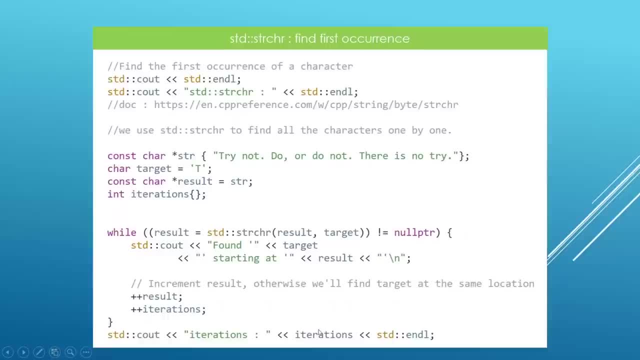 going to fail and we're going to fall down here and say how many iterations we found. i realize this example can be really confusing. i am going to try and explain it again. when we hit visual studio code for now, know that this facility can help you find characters in a string. that's the. 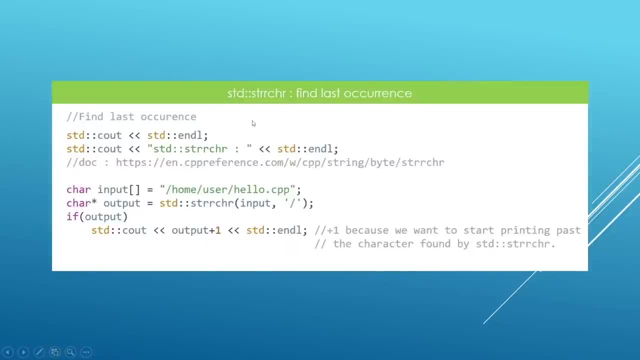 message here. there is also another function that helps you find the last occurrence of a character in a string, for example. here we have a character input- it is a path to a file on some limit system or map system- and we have an output character pointer which is going to store. 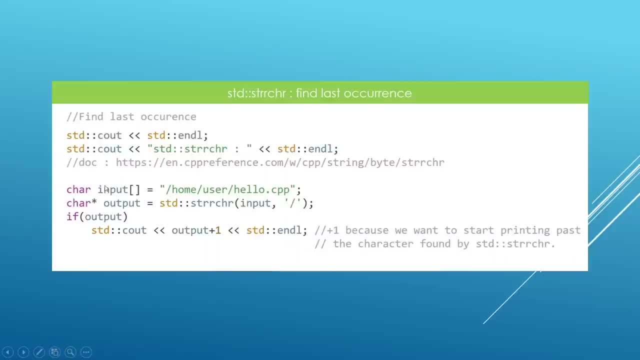 the pointer to the character that we found. okay, if we find the character, we're going to store in the pointer to that character. if we don't find it, we're going to return no pointer. i think that's how this thing works. so what we really want here is to hunt for the file name in this path here. 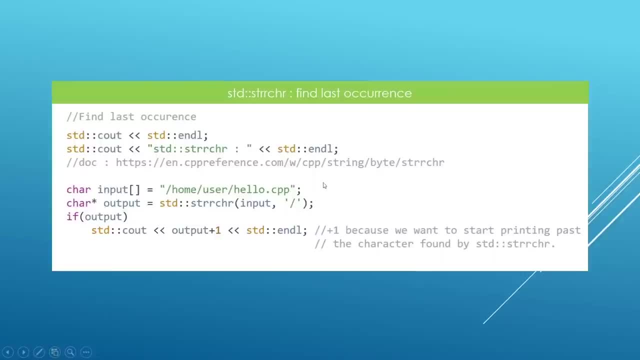 and this is really interesting. so we're going to search for the backslash, the last one in this string here, and it is going to find this guy here, because that's the last occurrence of the backslash in our input string here. once we find it, we're going to get. 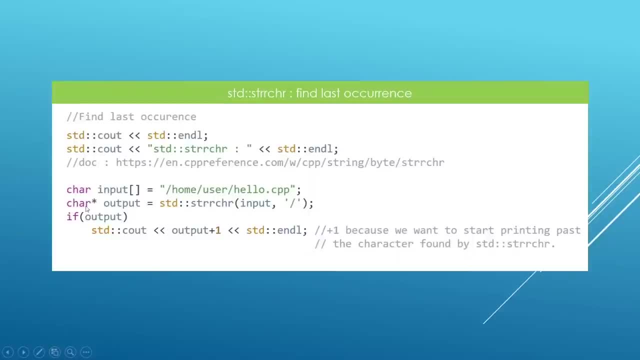 a pointer to this guy, stored in the output character pointer here, and we're going to print it out. what we're going to do? we're going to use pointer arithmetic to move this pointer to the next guy, because that's what we really want. we want to print, starting from the h here, and that's. 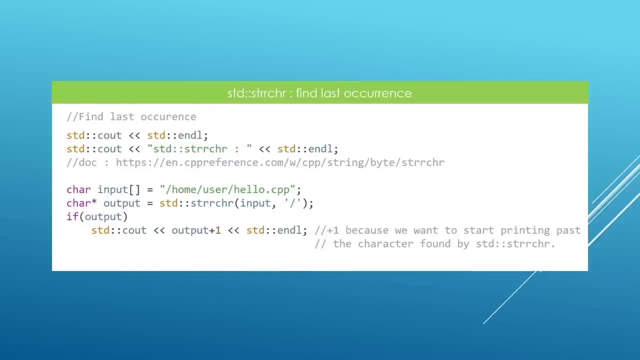 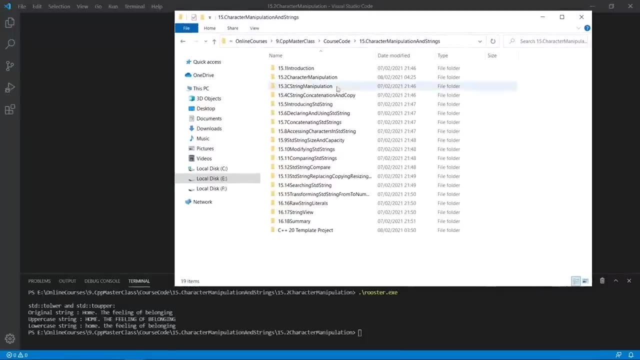 now that we have looked at all these examples, i think it is time we headed to visual studio code and actually played with them. okay, here we are in our working folder. the current project is c string manipulation. that's what we're going to work on. we're going to copy our template files. 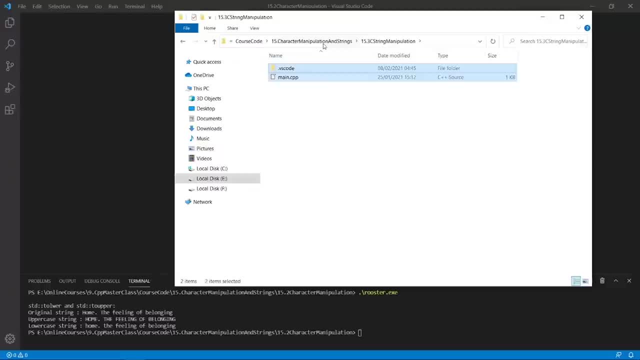 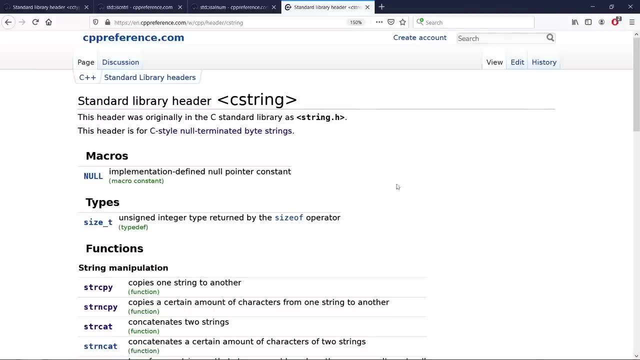 and we're going to put that in place and we're going to open this in visual studio code pretty quick. let's include c string, because that's what we're going to be using. many of the things we're going to be playing with in this lecture are documented in this piece of documentation here. 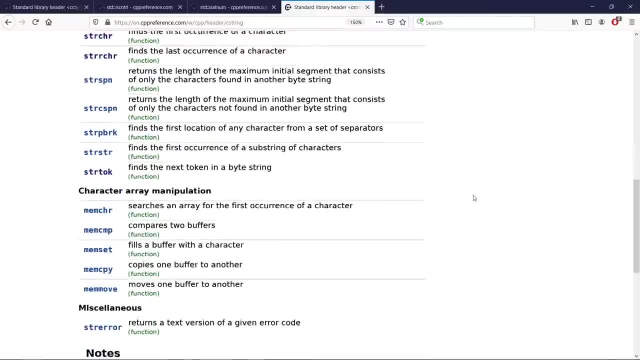 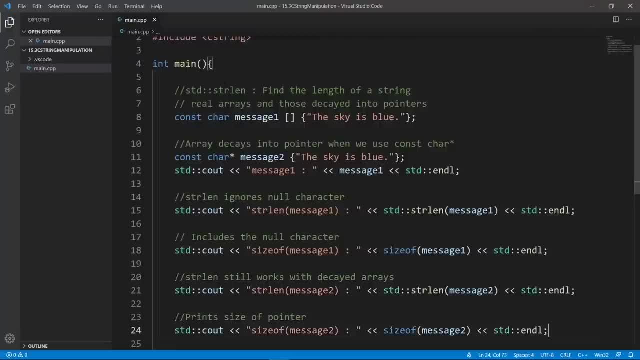 so you can come here and get more details than we could even cover in a course like this. let's bring this up a little bit and we're going to go in our main function and put in the first piece of code we can play with. the str lan facility is going to find the length of the string and it's going to 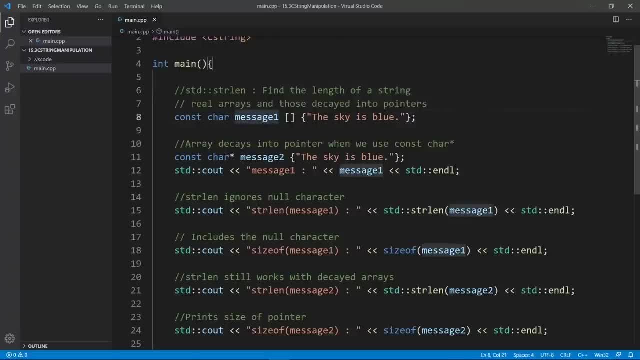 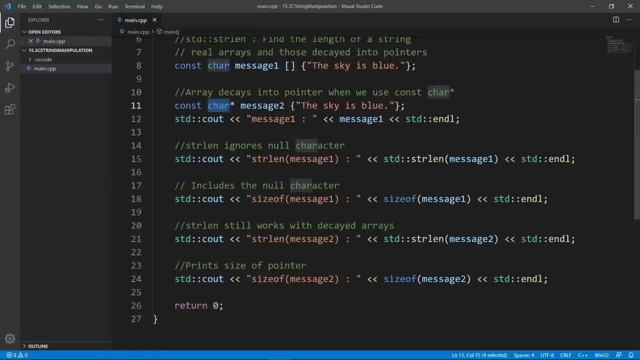 work, regardless of whether you are using a row array like this, or even if you are using a character pointer to point to the point of the string, and you're going to be playing with this, your array, and this is pretty cool. so here we have strlen message one. we're going to print that out. 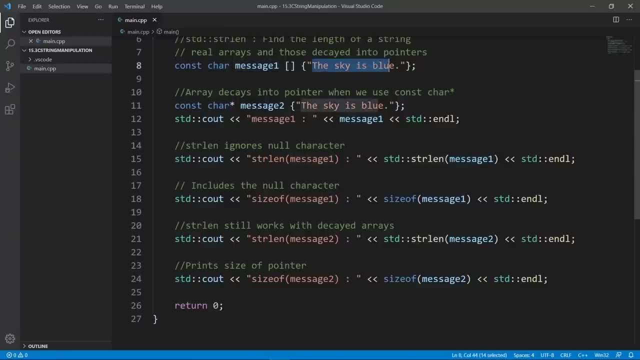 we're going to print how many characters we have in this guy here. we're going to also use the size of operator to try and compare these things. but please know that the null character is going to be included if you use size of here on a row array. this is very important to know. but one 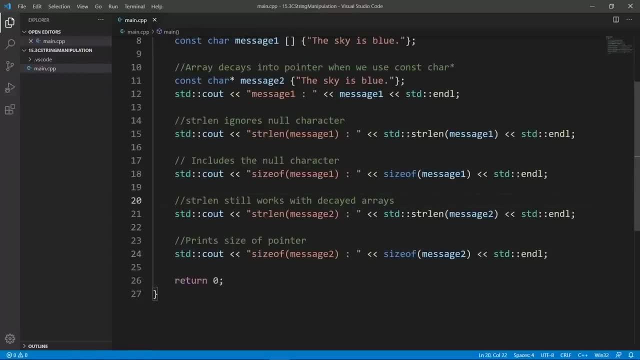 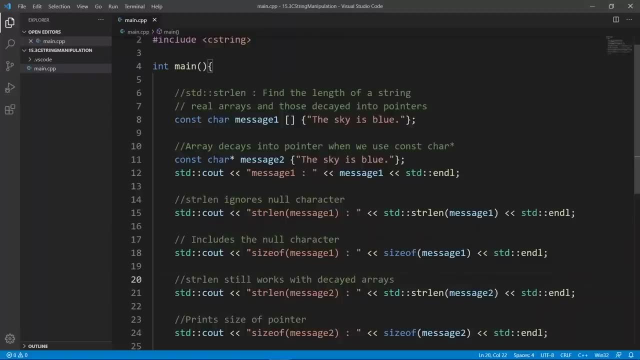 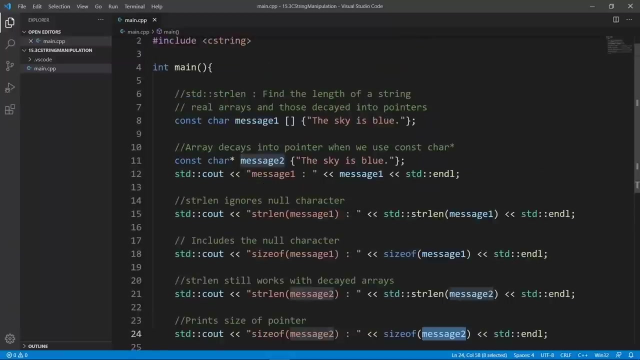 interesting thing about strlen is that it is also going to work if you are storing your array and something that is pointed to by a pointer. so even decayed pointers are going to be usable here, and this is pretty cool. so we can also try and print the size of message 2, which is pointed to. 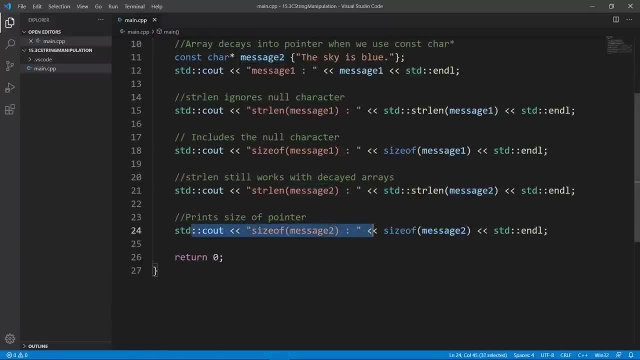 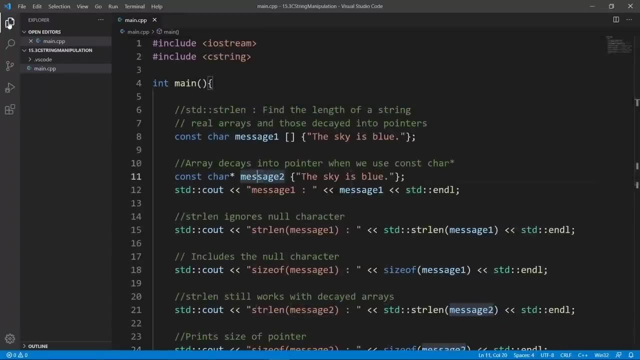 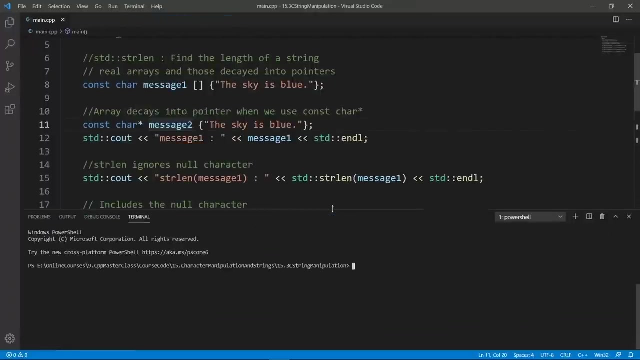 by a row pointer and we're going to see what we get, but we know that we're going to get the size of a pointer, because that's what it really is. message 2: here is just a pointer. okay, let's close this on the left and we are going to bring up our terminal and try and build this with gcc. we're. 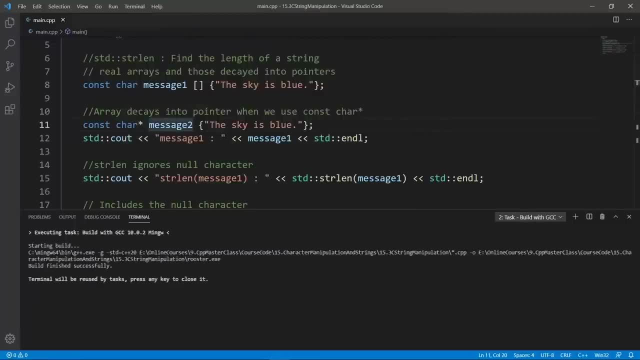 going to do that. so we're going to use gcc to build this. the build is going to go through and we're going to clear and run rooster again and this is going to give us what we want. strlen. message 1 is 16. size of message 1 is 17 because size of is also going to count, the null character strlen. 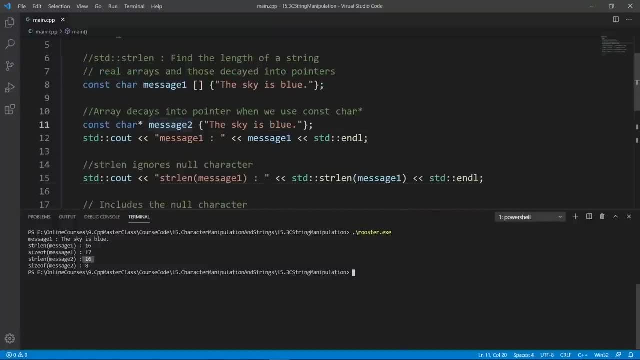 message 2. you see that it works even if we have a decayed array that is pointed to by a pointer, and this is really useful. if you happen to need the size of an array like this, you can use strlen and you're going to get the size of data in there, but know that the null terminating character is not counted if you use 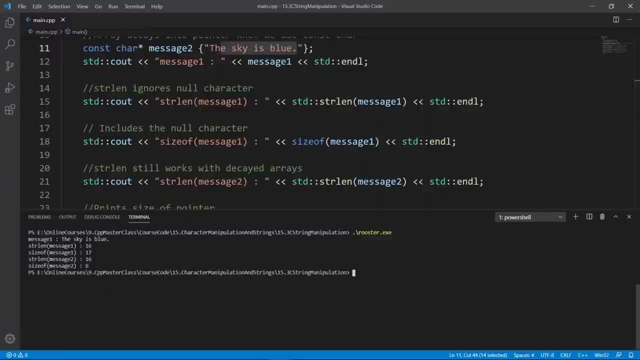 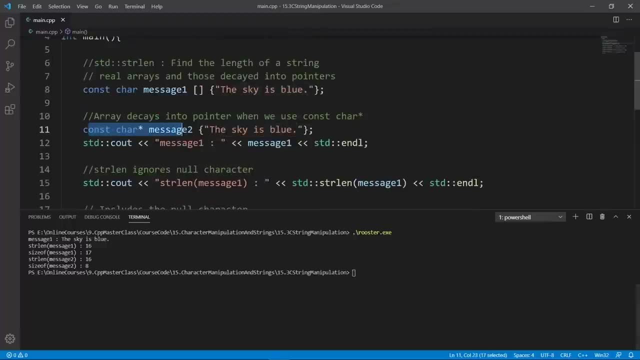 strlen here and size of message 2 is going to be 8 because that's the size of a pointer on our system here. so know that this guy is going to be 8 because that's the size of a pointer on our system here. so know that this guy is just a pointer. okay, that's the message here. we are going to comment this out. 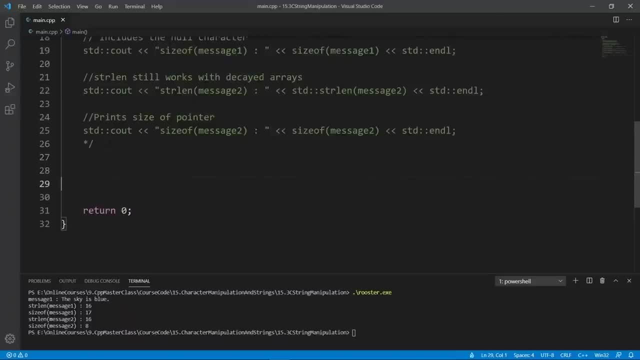 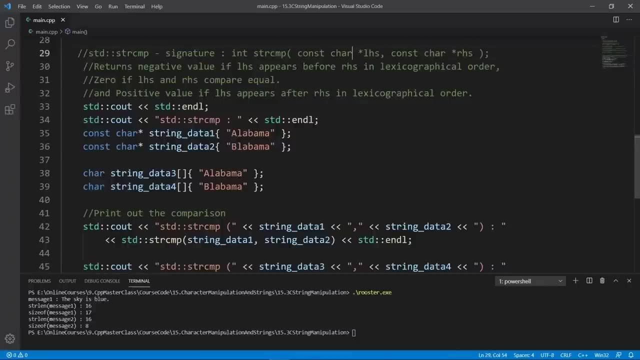 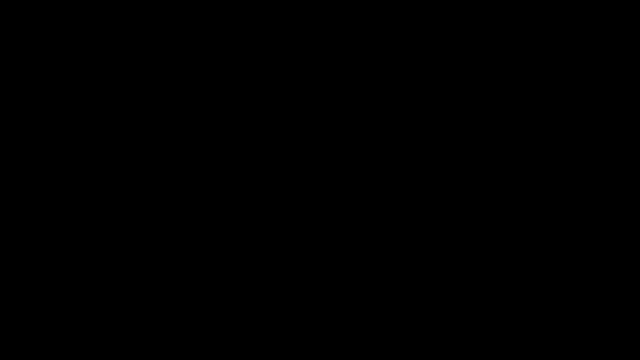 the next thing we're going to look at is strcmp, which can be used to compare strengths. so it works exactly like we say. it's going to return something negative if the first strength happens to come in front of the second strength in lexicographical order. so we could say that is by 0. mattered, but this would depend on thesna baby. 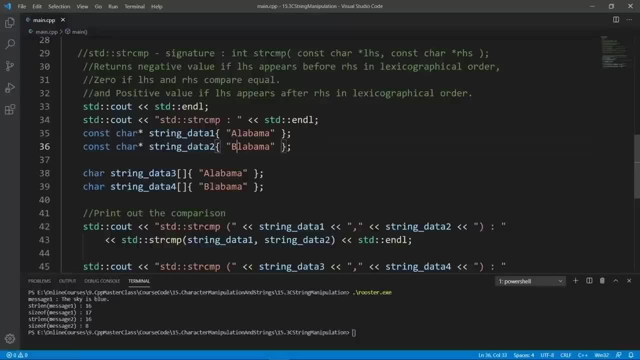 because string by has strength anyways. whatever do we want to identify now the- by missing something to show the lots ofман heading only g x, gu, for example. here we have a few variables. we have Alabama and Alabama. there are strengths pointed to by pointers. for example, here we have a few variables. we have Alabama and Alabama. there are strengths pointed to by. 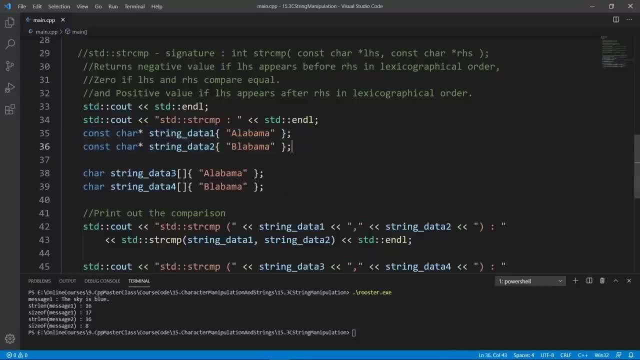 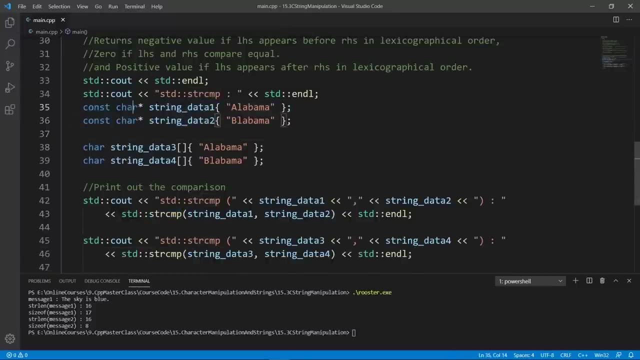 pointers. for example, here we have a few variables, we have Alabama and Alabama. there are strengths pointed to by pointer o. further stretching string string array or your C string is stored, so we're going to use that here for our C string pointer. two: by pointers we're going to try and compare whatever is in string data one with string data two string. 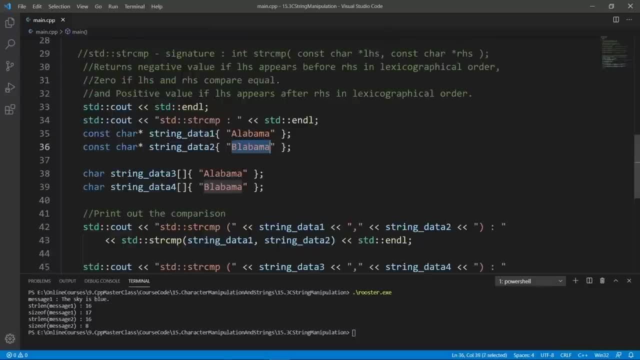 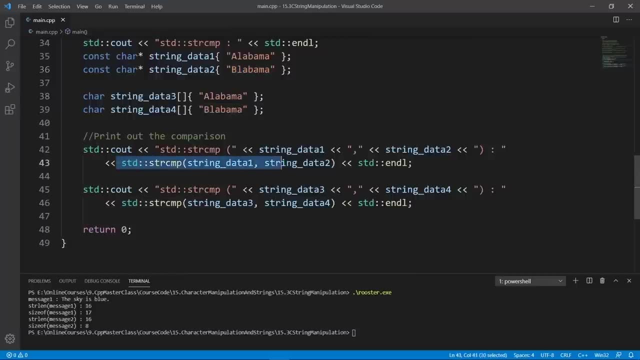 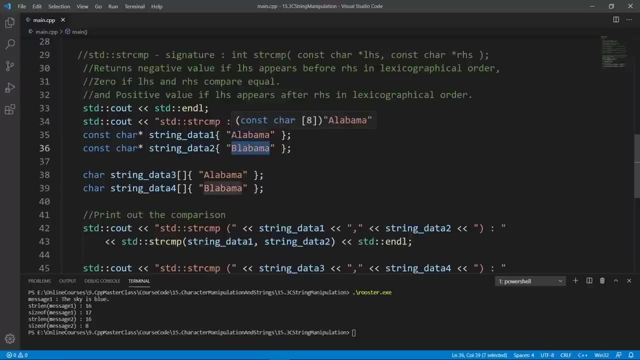 data one has Alabama string data. two has blah Bama. so if we compare these guys, we expect to get a negative value out of this thing here, strcmp, because Alabama comes in front of blah Bama in our alphabet, so a is in front of B. so we're going to get a negative value out of this and we expect to. 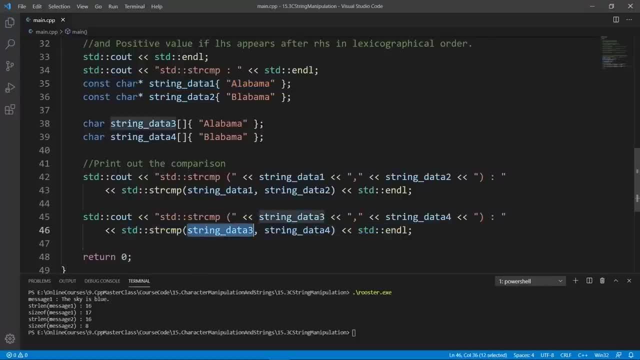 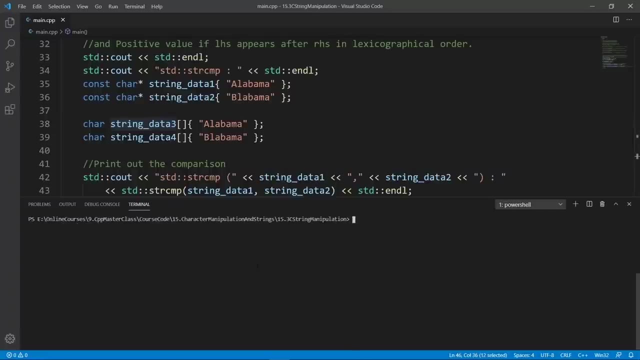 get the same thing in the second example here, which is going to be using what we store in our row array. so make sure you understand this and we're going to try and build this to see that it passes through our gcc compiler. the world is good. so we're going to clear and run rooster and you're going to see. 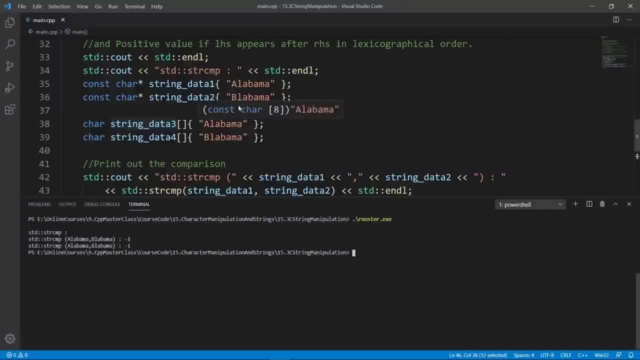 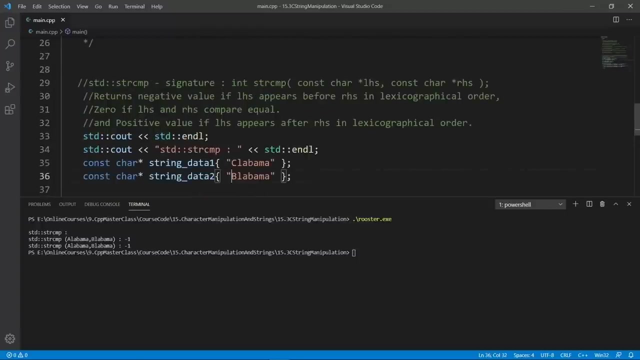 that we get a negative one. I want you to play with this thanks, and try and change, for example, the a to a c and see what you get. okay, we're going to try and build, but before we do try to expect to see what you get. C comes after blah Bama, so if we look at this description here, we should get: 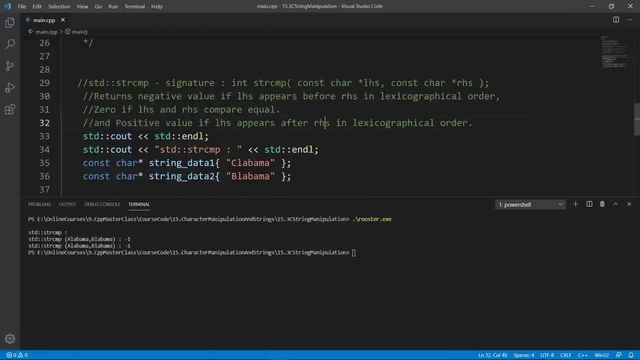 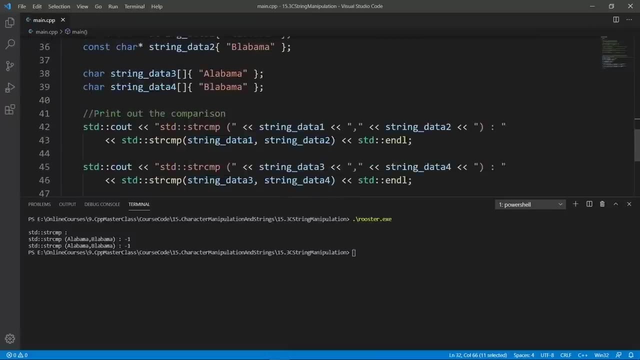 a positive value because the first guy comes after the second guy in the lexicographical order, so we should get a positive value for the first thing that we print here. okay, let's work and see if that's the case. we're going to build successfully, we're going to clear and run rooster and you see that the first 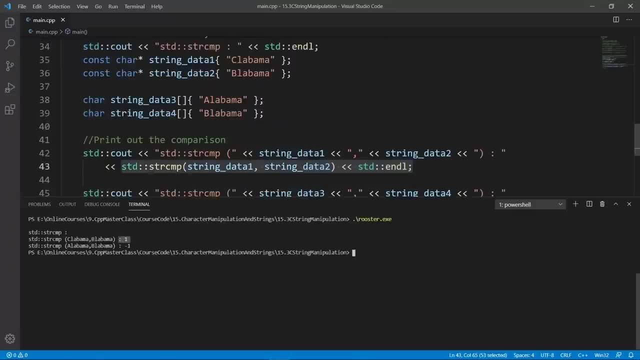 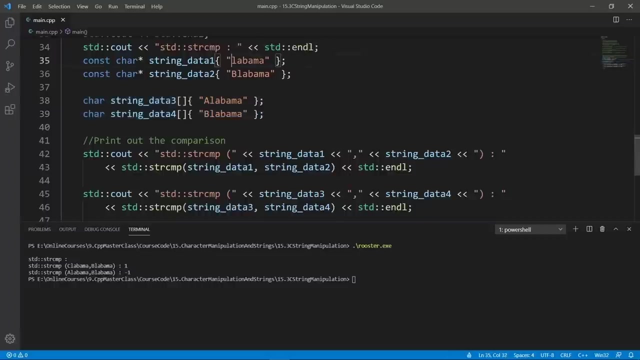 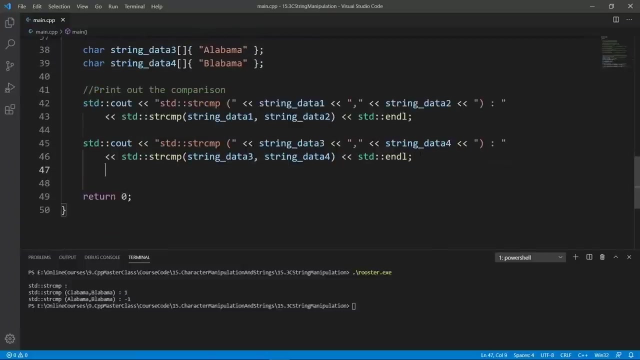 guy prints a one because lagama comes before blah Bama and the second one is going to still be a negative one because we still have whatever before in there. okay, this is how you work with this, thanks, let's turn this back to alabama so that we are not confused and we're going to keep working on this. and the next piece of code. 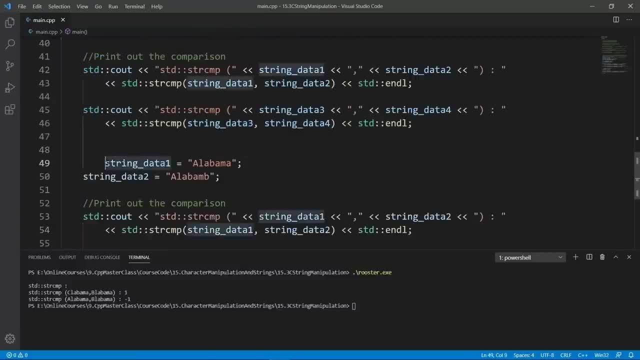 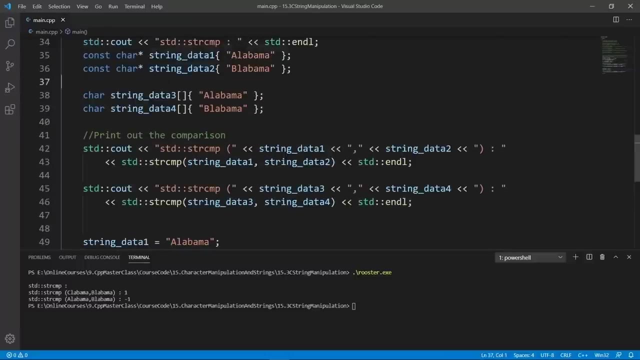 we are going to try and modify whatever is stored in string data 1 and string data 2 and print the comparisons out. for example, we have alabama and alabam and, by the way, we are able to modify that because it is a pointer to a string and notice that this is not the const pointer. so we can. 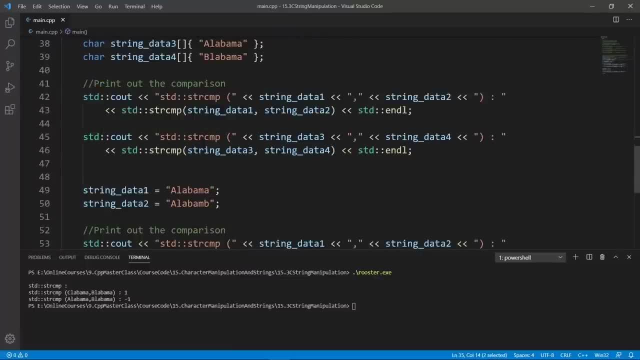 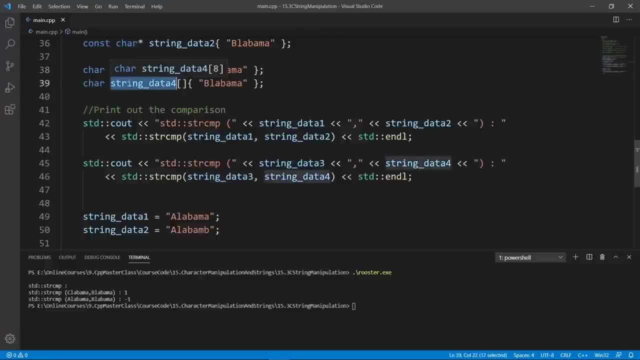 really change where this guy is pointing, and that's what we are doing here. but we can't do that with string data 3 and string data 4 because these are arrays and, remember, you can't change where an array points. so this is going to compile, nice. but if we try and do the same thing with 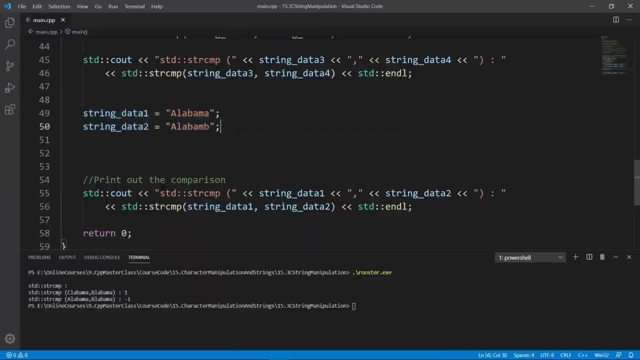 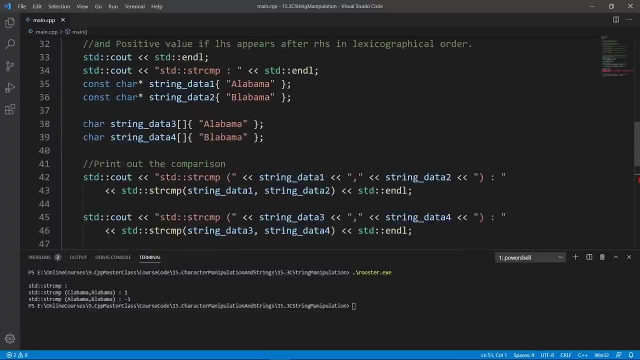 string data 3 and string data 4. let's do that. you're going to get a compiler error. so we're going to put this guy here and say 3 and 4 and we should see visual studio code complaining here, because this is not allowed. you're not allowed to make an array point to 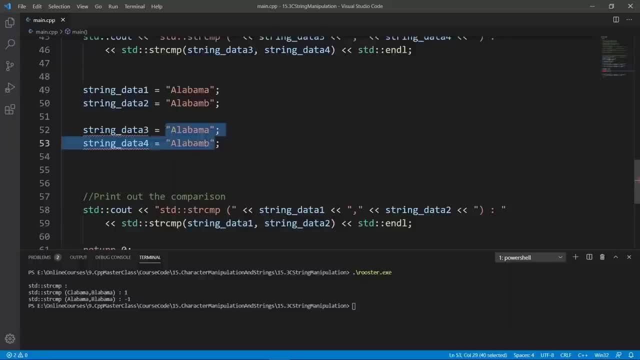 another location and this is just another character array or cost character array in memory that we want this pointers to point to, or this array to pointer, and this is not possible. so we're going to get a compiler error if we do this. this is something i wanted you to know, that's. 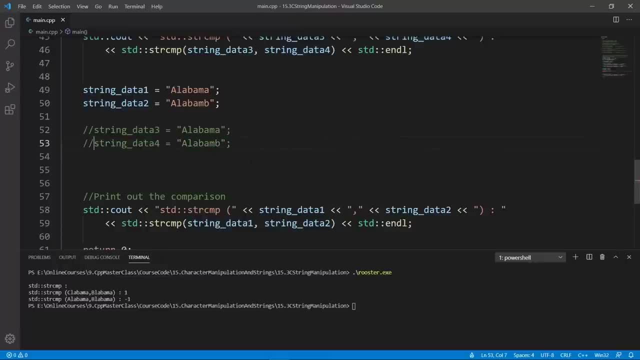 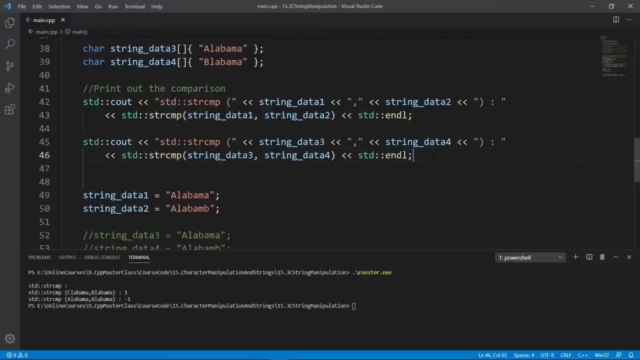 why i set up this example here. so if we run this, we're going to see the first line of output here, or i think i should comment that out, or let's not comment it out now. if we run this program, we're going to get the output for alabama. 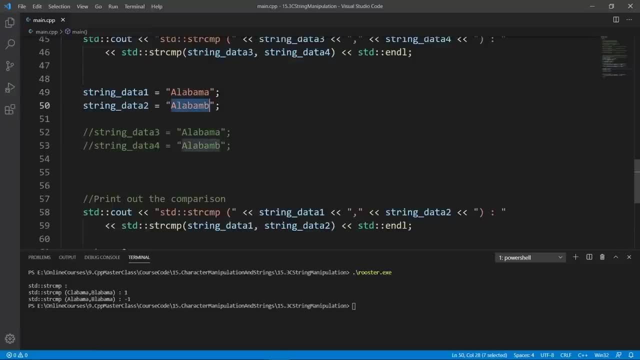 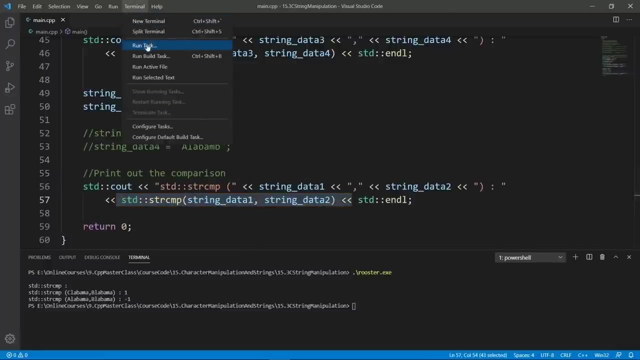 and alabama printed out and alabama comes after alabama. so we expect to get a negative one, because the first guy here comes in front of the second guy, so we're going to get a negative one out of the think we are doing here. let's try a world with gcc. the build is going to be good, so we're. 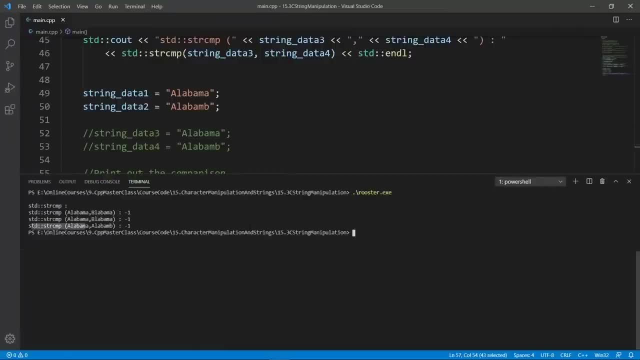 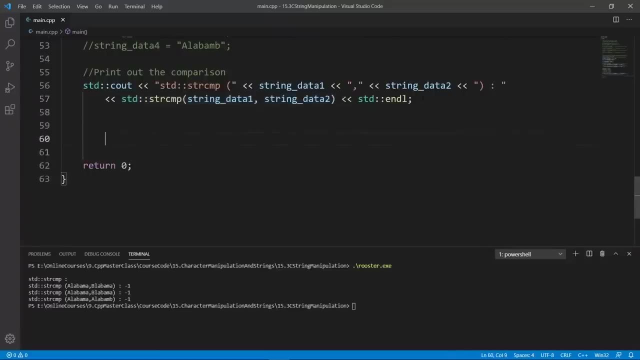 going to clear and run rooster and we're going to see that we have a negative one here. alabama comes in front of alabump, so this is cool, so we can try and put in many other examples for you to play with. i am going to do that because i don't want to type all these things. 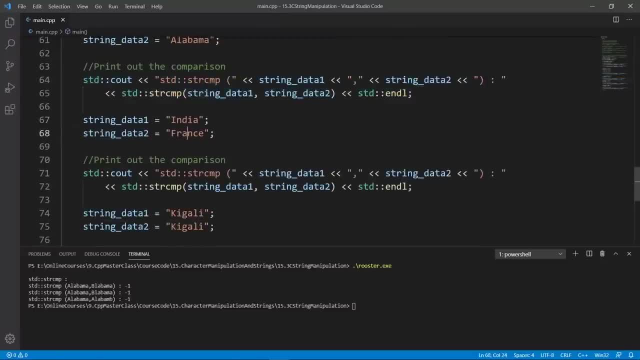 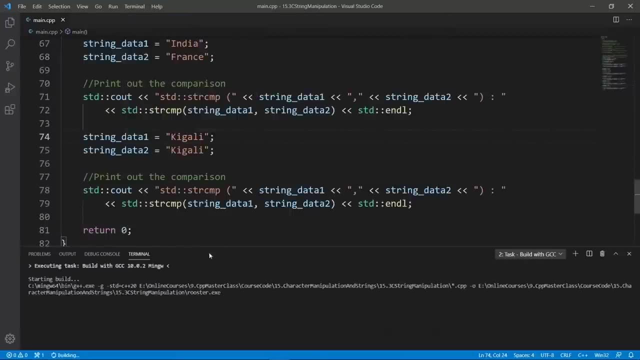 and we're going to print the result out. for example, we put in india and france, we put in kigali and kigali and we're going to get things printed out here. so let's build this so that we don't waste time. we're going to clear and we're going to run rooster and we're going to see that. 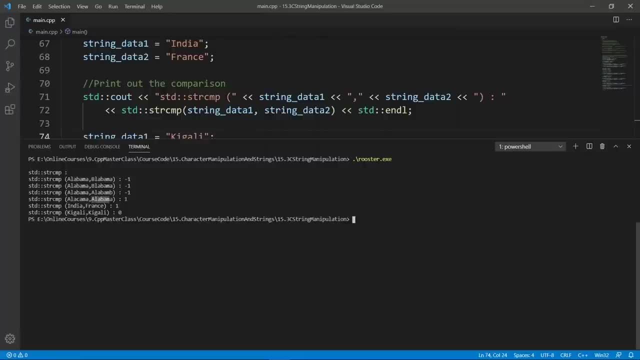 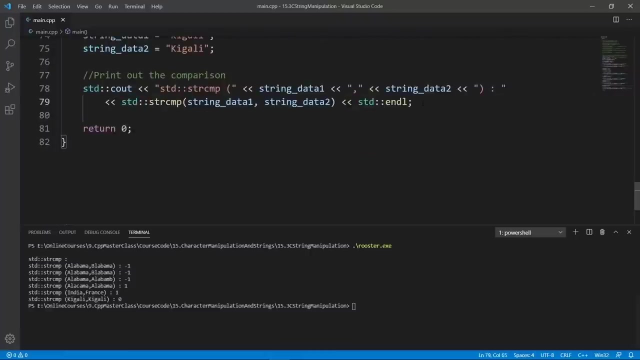 we get these things here: alakama comes after alabama, so we get a one. india comes after france, we get a one. kigali comes together with kigali and we get a zero. you can try and put in whatever you want. these are just a few examples for you to play with, and by now i hope you really. 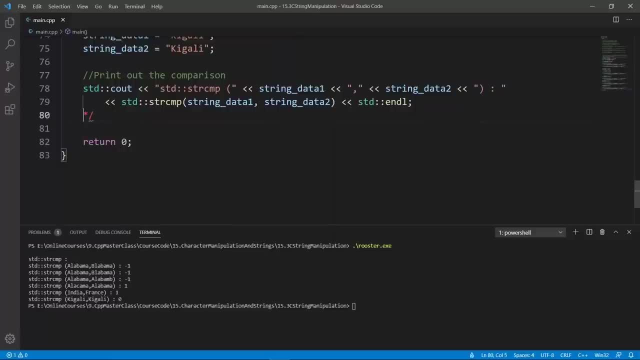 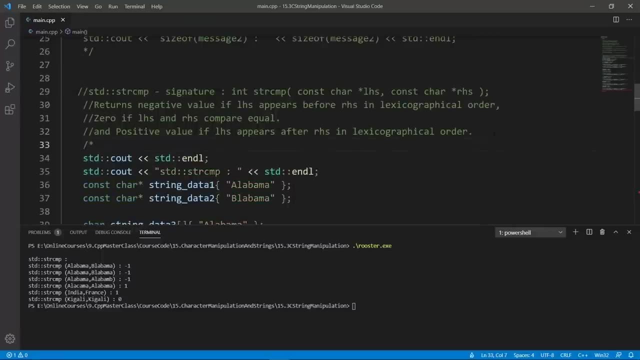 understand how this function works or this facility works, so we're going to comment it out, whatever we did here. so we're going to comment all this out so that we don't have noise output in. whatever we want to do next and what we want to look at next is this function here, which is: 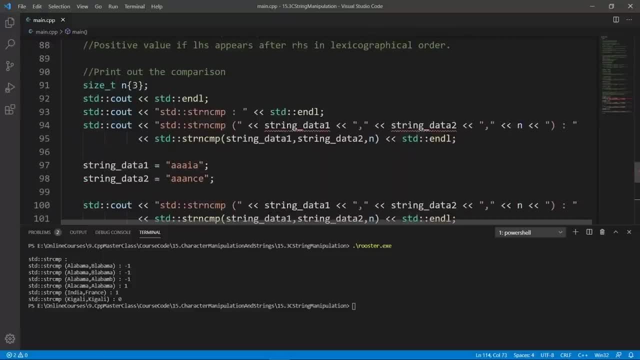 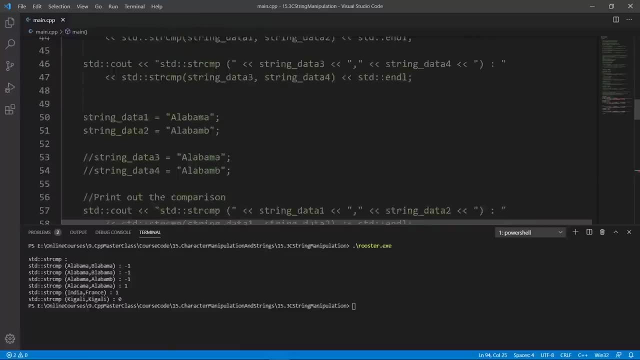 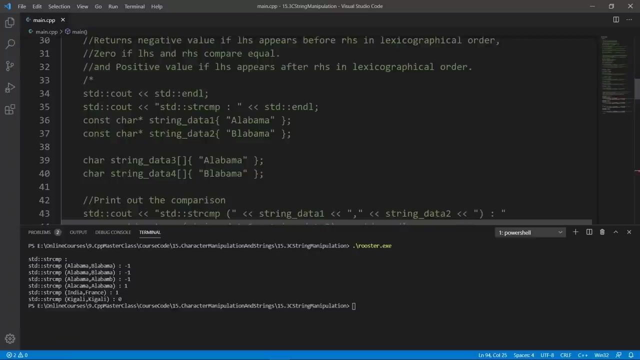 going to compare strings in the same ways, but we're going to tell it to compare however many characters in the string and you see that my string here has been commented out. i can quickly take it and bring it down here. let's do that. i can't find that. let's find that and copy it down and we're going to find. 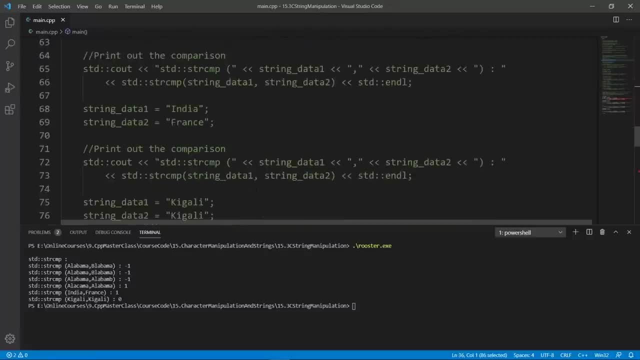 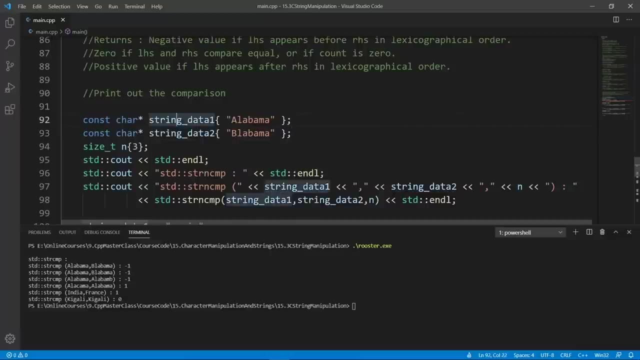 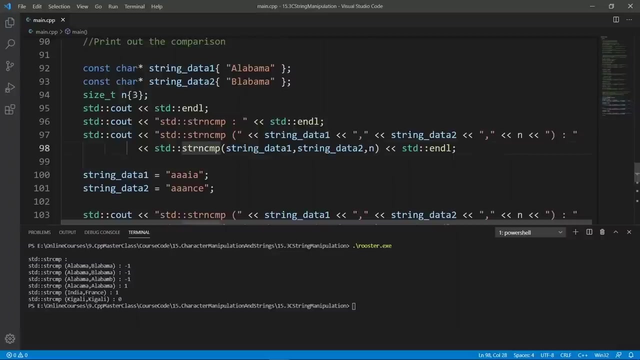 them here. so i'm going to find this and bring that down here so that i can compare these things. so let's come down here and print and put in our declarations for these strings and you see that visual studio code is happy now. so what we're going to do is compare a set of characters in. 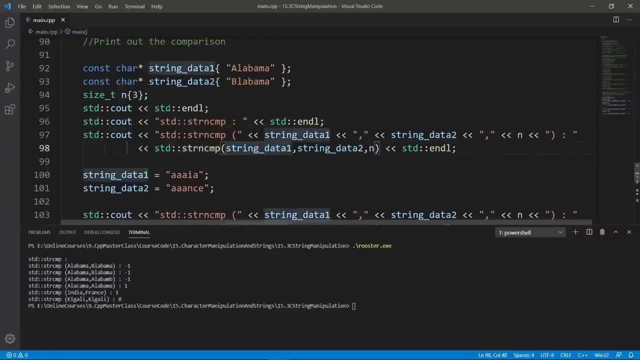 these strings here. okay, so we're going to compare any characters in our strings, so we're going to compare ala to blah here and ala is going to come in front of blah, so we're going to have a negative one printed out here. but if we change the strings, 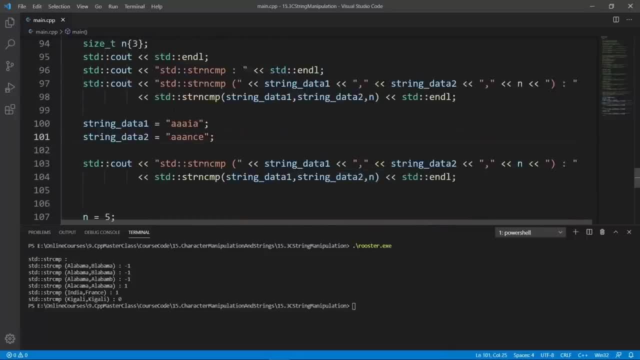 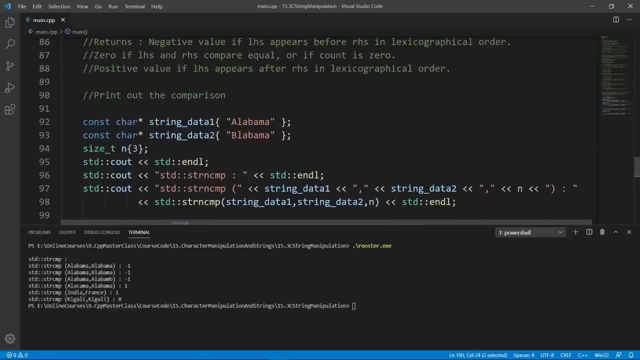 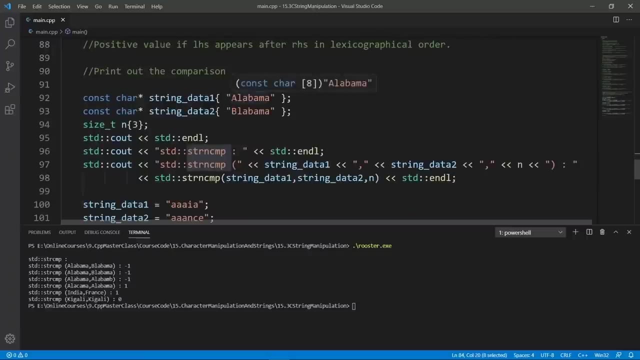 to aaa and aaa here and compare the first three characters. we're going to get a zero printed out because the first three characters are equal. and again, the special thing about this function is that it allows you to specify a number of characters you want to compare in these two strings. so you can say i want to compare three strands. you can say i want to 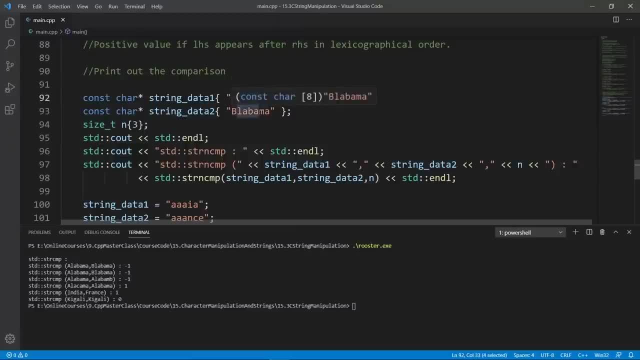 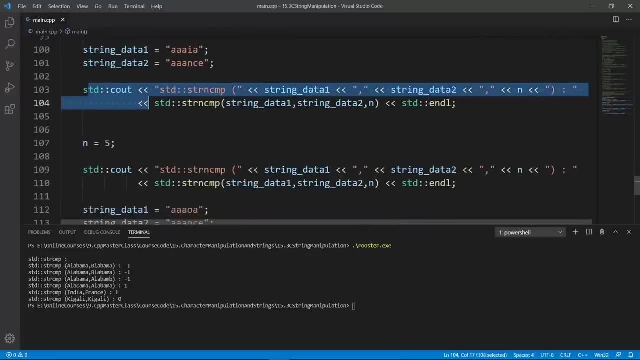 compare four strands or five, just make sure that you don't go over the size of the strand, and if you do that, it's not going to make sense what you are trying to do here. if we go down here, we're going to change n to five and we're going to be comparing all these things in here and we're going 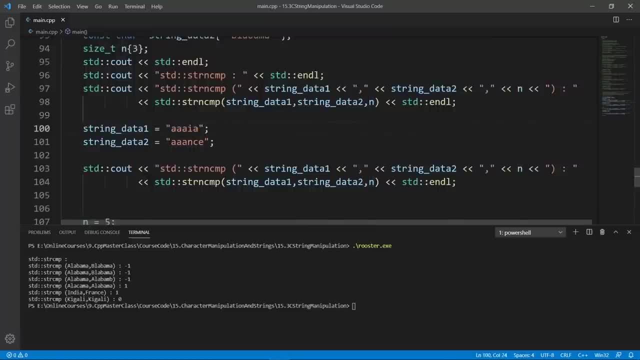 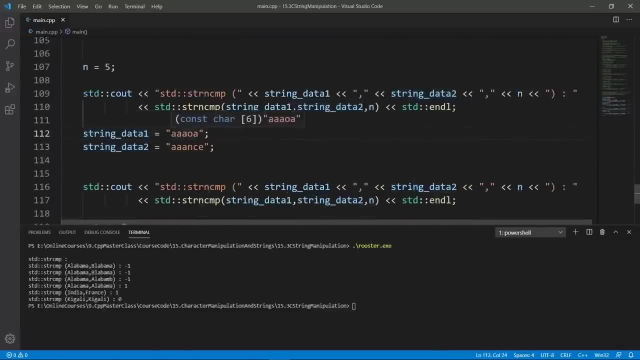 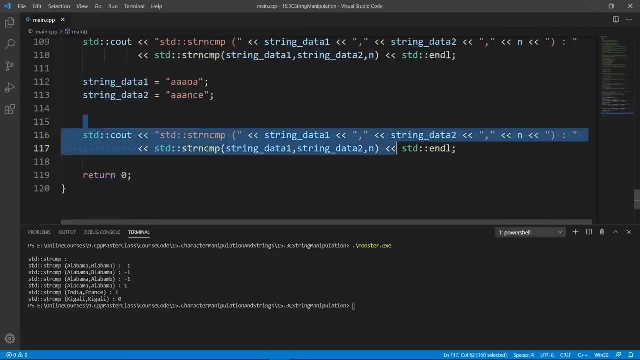 to get that. the first one comes in front of the second one because i comes in front of n in our alphabet. if we change the data to o here and n out is going to come after n and we're going to get a positive number printed out here. we're going to try and run this, so let's run the task to build with the gcc. 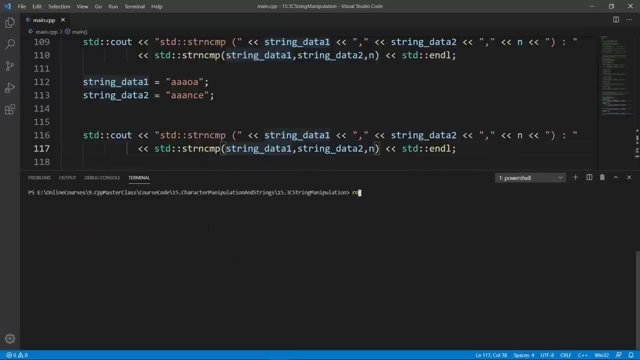 the build is going to be good and we're going to clear and run rooster and we're going to see that alabama comes in front of blabama because we are comparing the first three characters. if we have aaa in here, we compare the three characters. you're going to see that they are equal. we get a zero if we change. 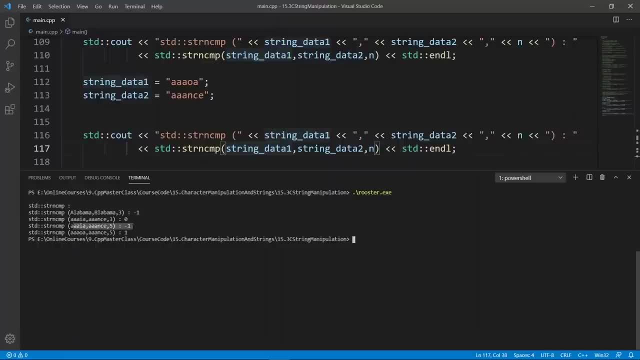 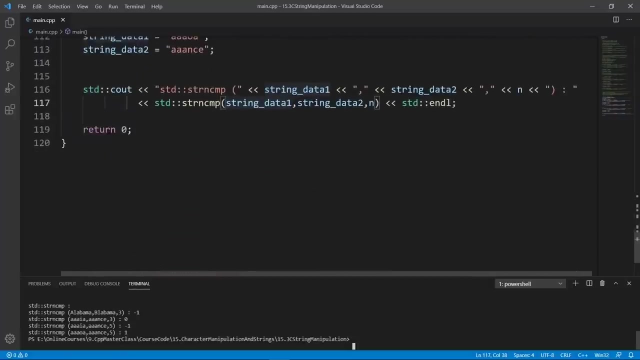 i and n here we're going to get a negative 1 because i comes in front of n. if we use o here and n, we're going to get a 1 because o comes after n. this is really simple to understand now that we know how to use the first version of string compare. this version is just going to allow us. 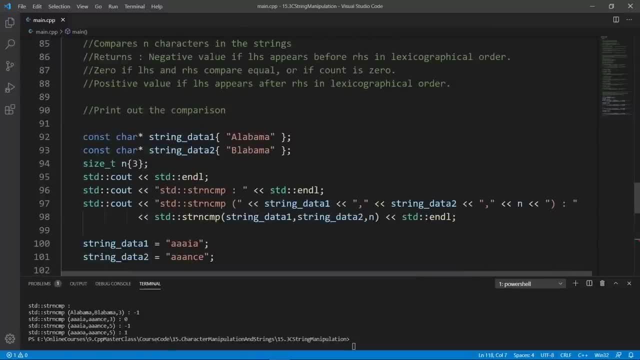 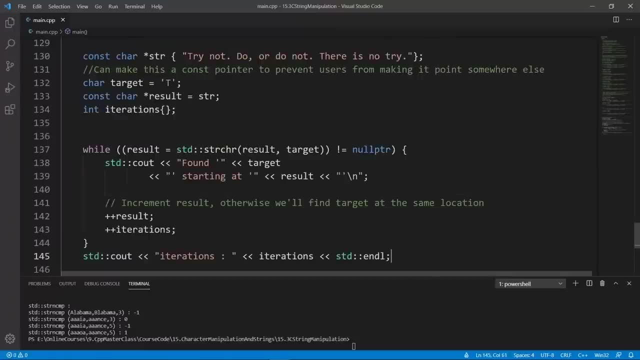 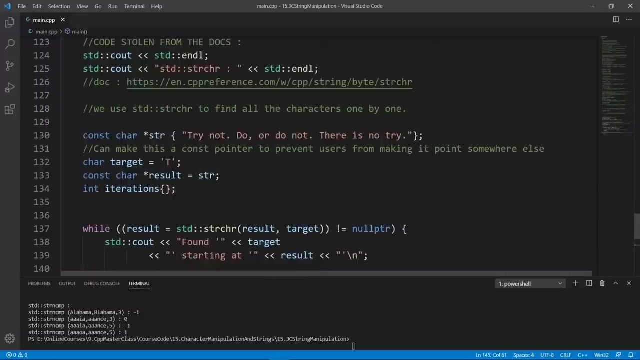 to specify how many characters in the string we want compared. so we're going to comment this out and we are going to go down and do another example that allows us to search for a character in a string and the method we use to do that is std, str, chr. so this guy is going to find whatever. 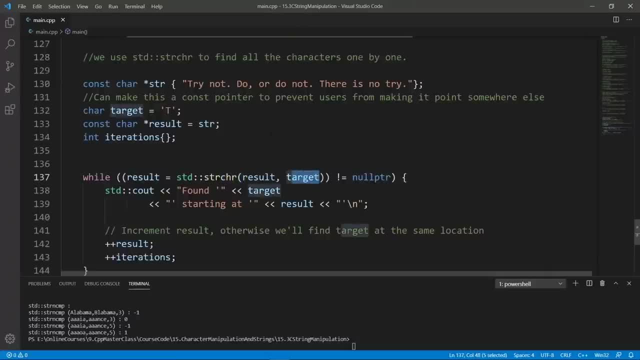 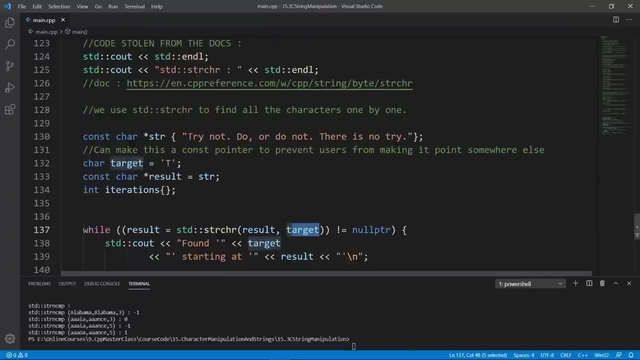 target you want to find and if it finds that, it's going to return you a pointer to dot target. if it doesn't find it, it's going to return you no pointer. so we set up an array here and we store that in a location that is pointed to by the pointer to character here and we say whatever target we are looking for. 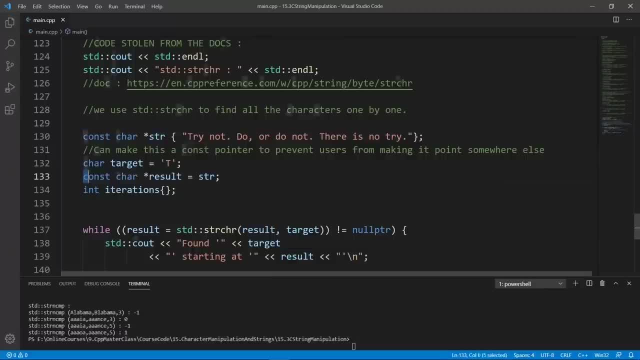 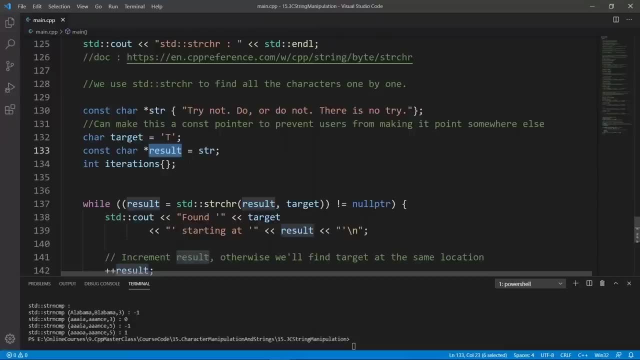 in this case we want to find this t. here we are going to set up another character array that is going to store our result. the result is really going to be a pointer, which is going to be pointing to something valid if we find the target, and it's going to be no pointer if we didn't find the target. 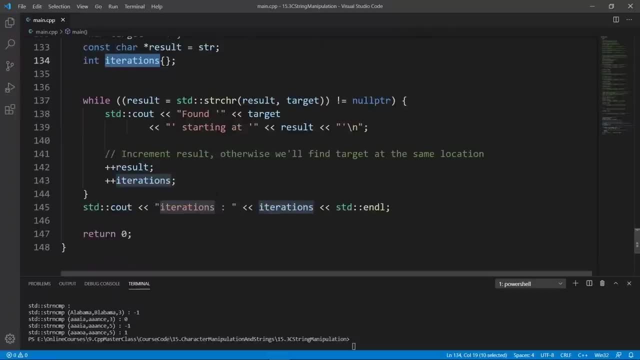 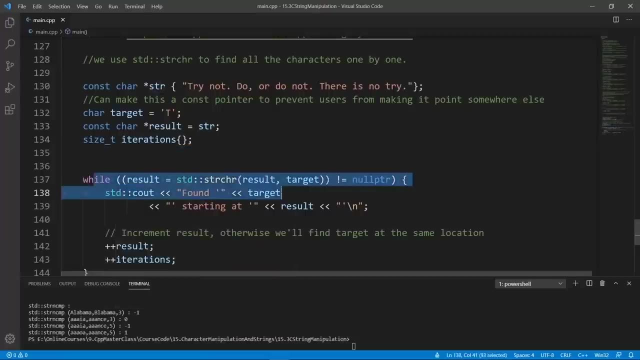 and we set up another variable which is going to store how many iterations we did. we should really make this an unsigned integer or size t. so let's make that here and we're going to loop here. so the first time we loop in here we're going to call this guy. we're going to say: i want to find a t. 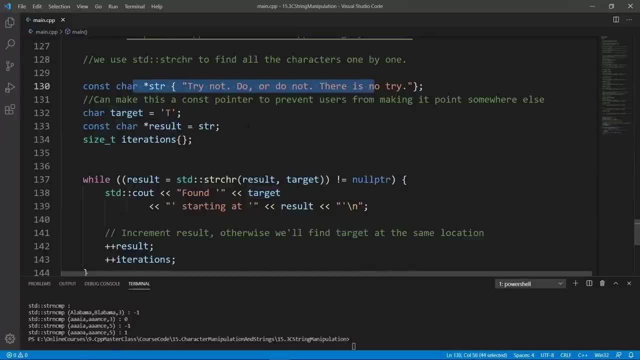 and resort here and the result is going to be pointing to this thing here because we did the assignment here. so it's going to go in and try to find a t. it's going to find the guy here at the first index and the test here is going to succeed. 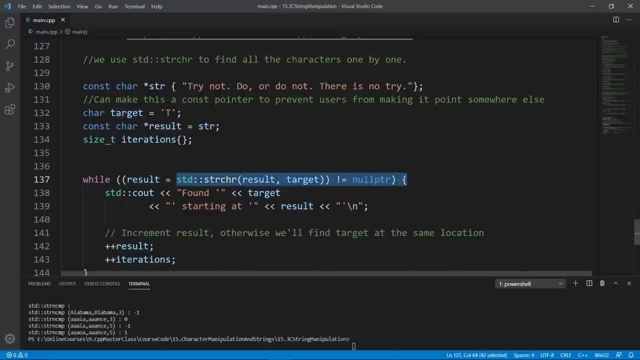 when it succeeds, it's not going to be equal to no pointer. it's going to be pointing to a valid pointer and it's going to succeed and return the pointer to be stored in resort. after this guy returns, the pointer is going to be stored in the research here and that's going to be a pointer to. 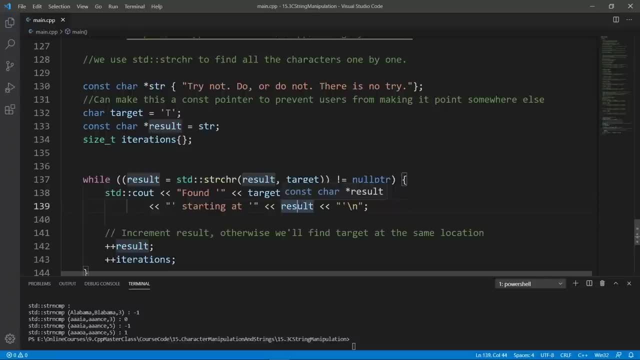 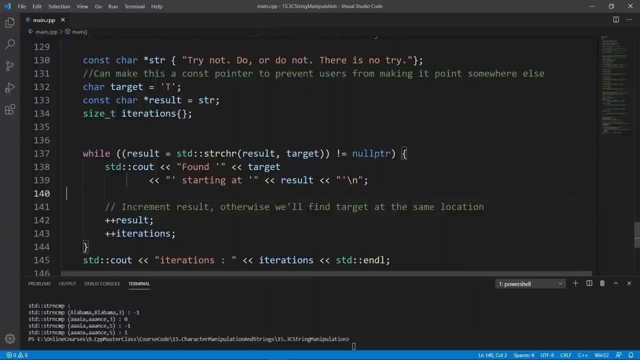 this team and we're going to jump in the body here. i really want you to understand how this thing is going to work. once we get in the body, we're going to say, uh-huh, we found our target. that's going to be our t printed out and it's going to start. 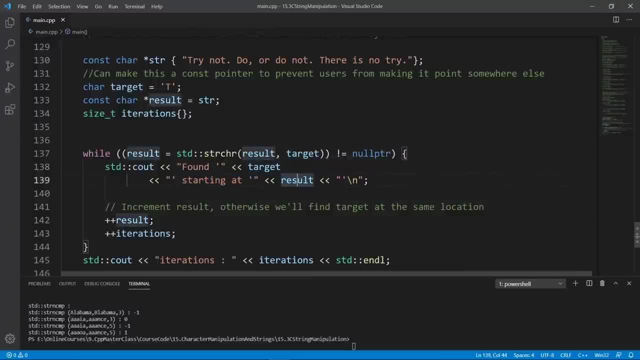 at this location. okay, and we're going to print, starting from the t here, because that's what our result here is pointing to. after we do that, we're going to increment the result to make it point to the next character. if we do that with pointer arithmetic, now we're going to be pointing. 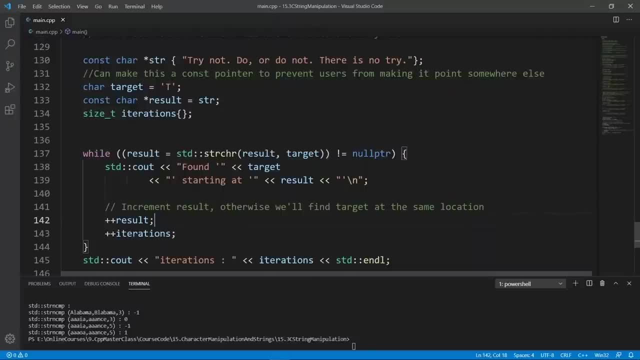 to the r in here. i hope this makes sense and we're going to increment our iterations. so we're going to say we have done one iteration and we're going to try and run this again and by the time we get in here we're going to have this string here in which we are searching for a t and it is going to be. 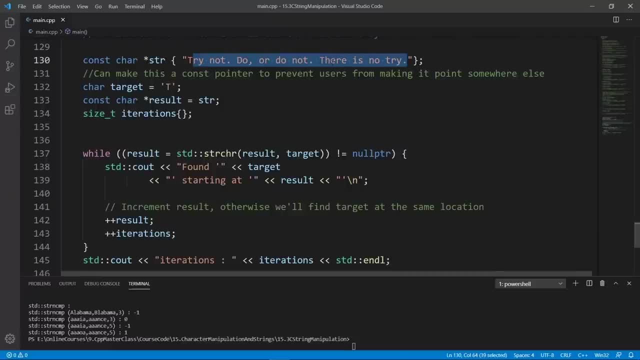 found, starting at this second t here, the there here, and it's going to find it. it's going to store the pointer to it to resort here, or i should say the search is going to be successful. so we're going to find the pointer to this t and return it from this function here and the pointer is going: 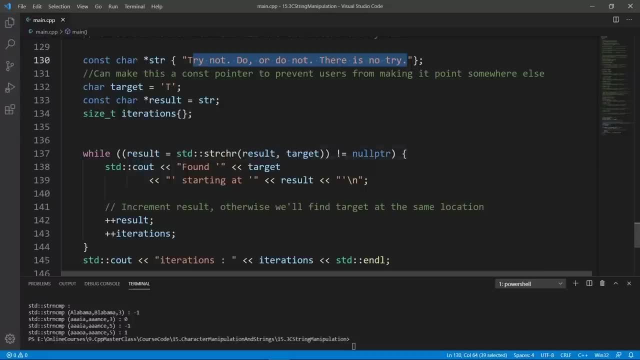 to be a pointer here. we're going to jump in the body and we're going to print. we found the target starting at this t. we're going to print that out and stdc out is going to print until it meets an old character. so we're going to print this thing through the end and we're going to put a slash n. 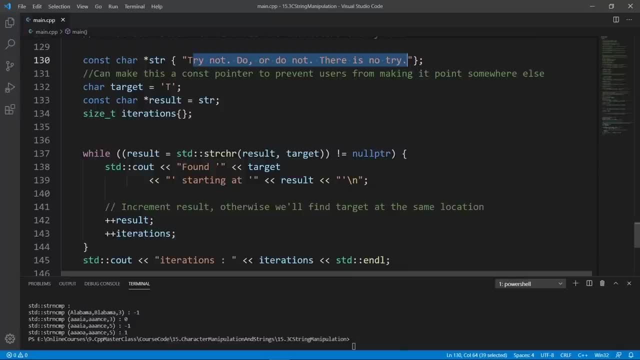 which is going to move us to the next line. after we do that, we're going to increment reset and uh, reserved now is going to point to the h here, and we're going to increment iterations. now we're going to have done two iterations by now and we're going to run the loop again. this time the loop is going to fail. 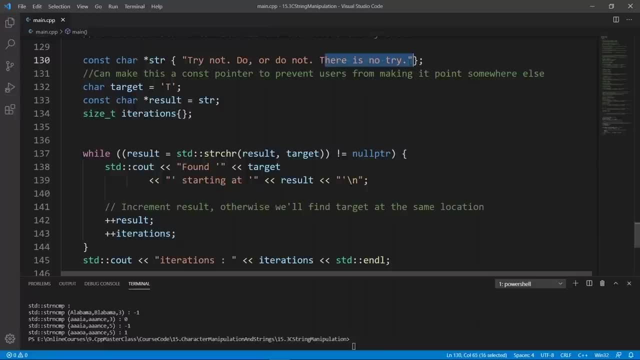 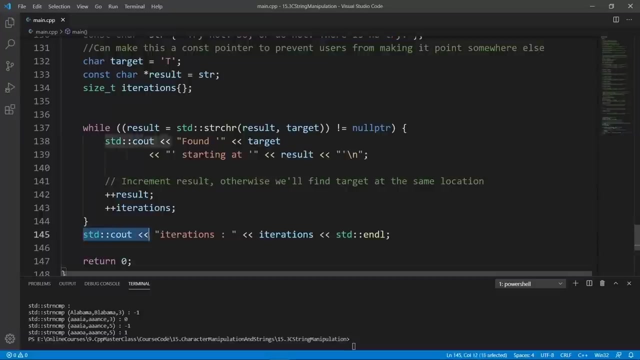 because, starting from here, we don't have a t and this function is going to return no pointer and this test here is going to fail. okay, we are going to return no pointer. no pointer is not going to be different from no pointer, so this is going to fail and we're going to fall down here and say how many. 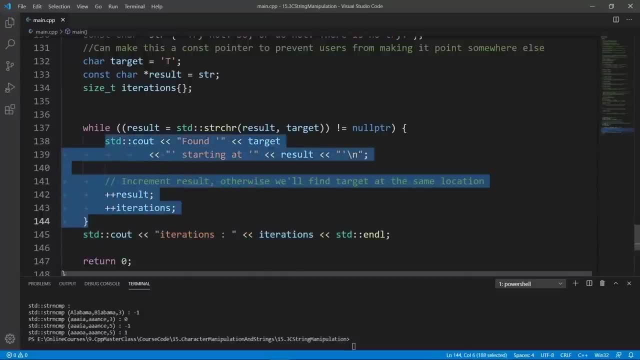 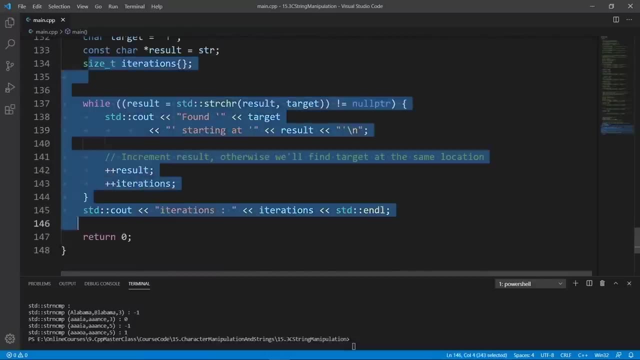 iterations we're going to find. so in total we're going to do two iterations and we are going to find two t and we're going to print whatever we find here. make sure you really understand this- and i put in this example on purpose, because it is a little complicated, but it is going to really 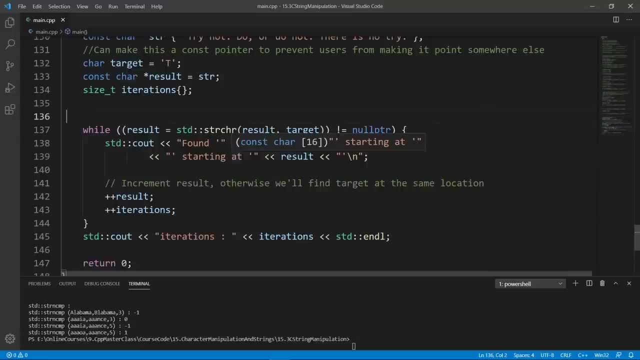 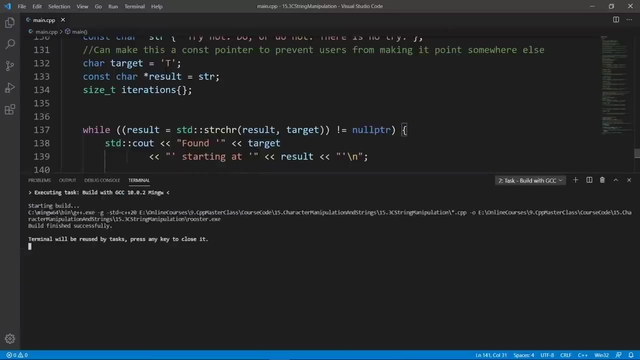 bring your game up in how you use these functions from the c++ standard library, and you really need to know this. if you have any problem with this, be sure to ask me. i will do the best i can to help you out. so we're going to build this and run this. we're going to build with gcc, as always, and we are. 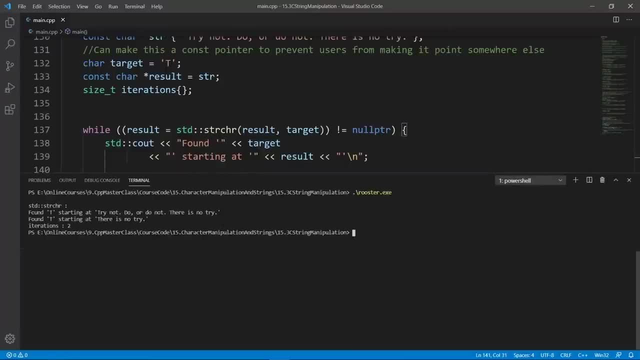 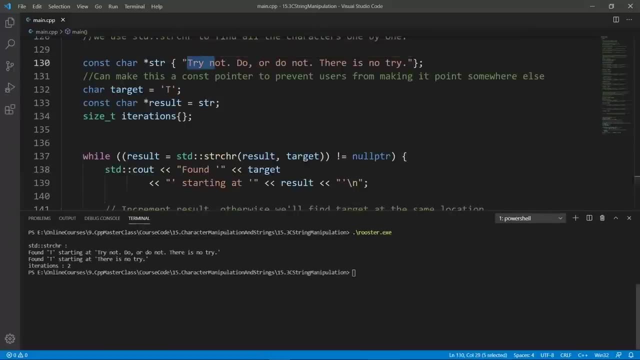 going to read a way to call this, i suppose in the reading of the internet. so let's see how this works. so we're going to copy this one into a word. we're going to show it to the computer, sorry, yes, we're going to copy this into gcc. so we're going to see that we are looking for another t. 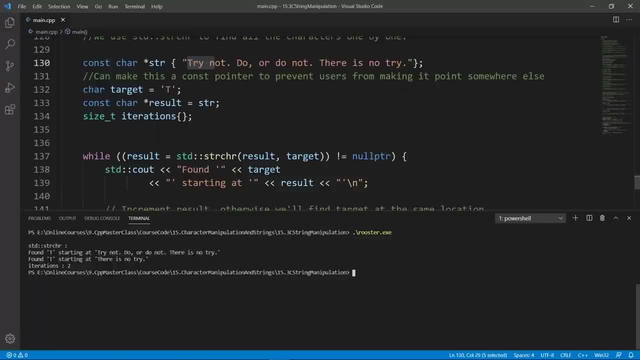 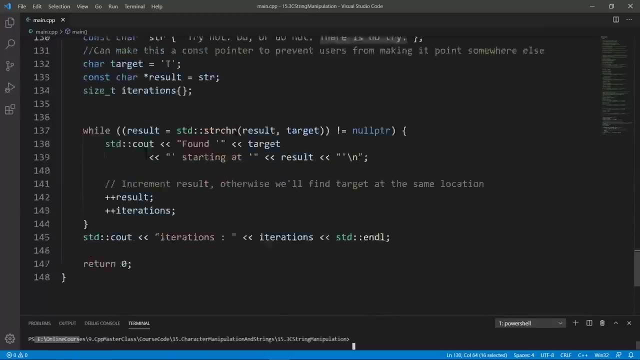 we are going to say: we found t starting at the t here. so we're going to say: try, okay, we're going to print all the message out and the second iteration is going to find t starting at this location here, and we're going to do two iterations in total. we're going to comment this out and again, if you. 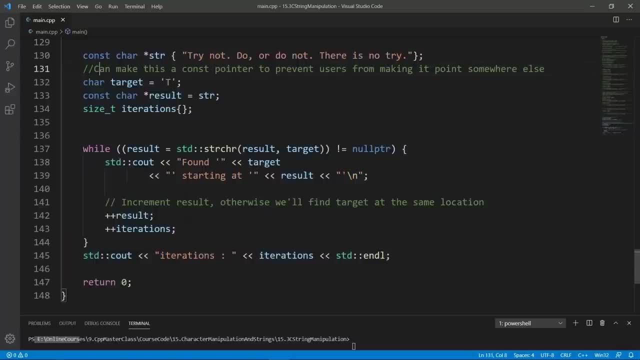 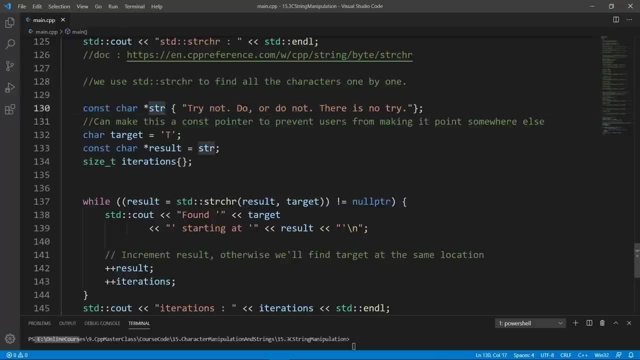 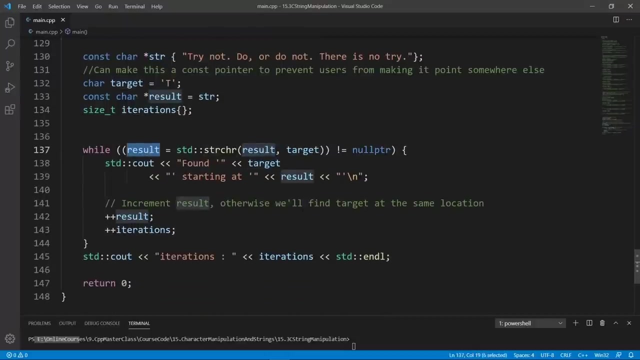 don't understand this. please go through it again best i can to help you out. and some of you might be asking: why did we go through the trouble to store this guy? in result: why don't we use htr in the first place? in here and the explanation i can. 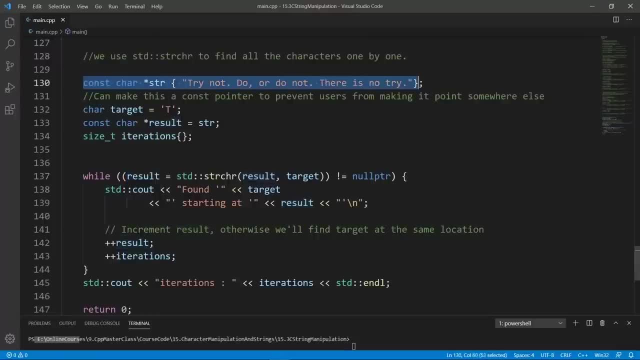 come up with is that you don't really want to modify this guy here, because somebody is going to look at this thing and say: this is the message i have in htr here. but if you try and modify this in the loop, it's going to be messed up because you're going to be incrementing it and doing all. 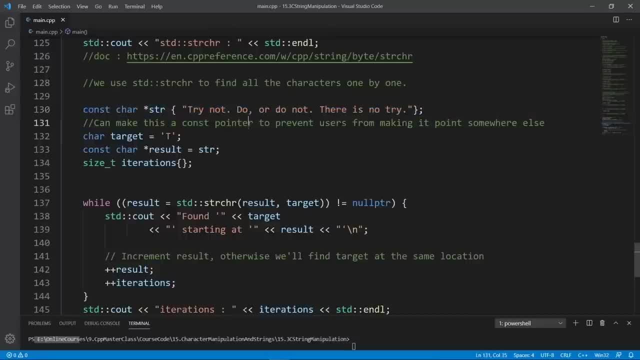 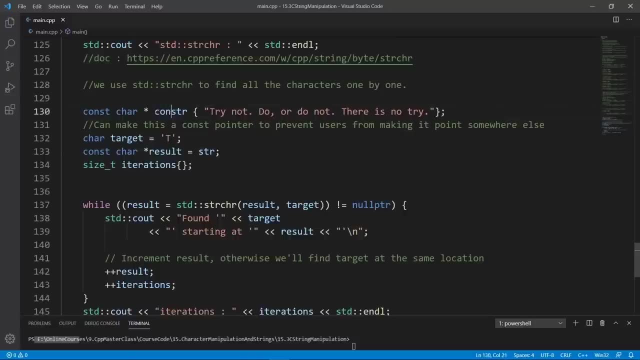 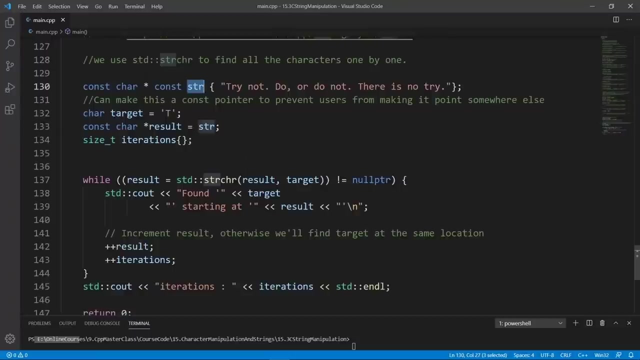 kinds of crazy things on it, so you don't really want to modify this. so a better way to even do this is to mark this as a cost pointer, and we know how to do that. so we can say cost here. and if you even try to increment htr somewhere you're going to get a compiler error. so let's make sure we see. 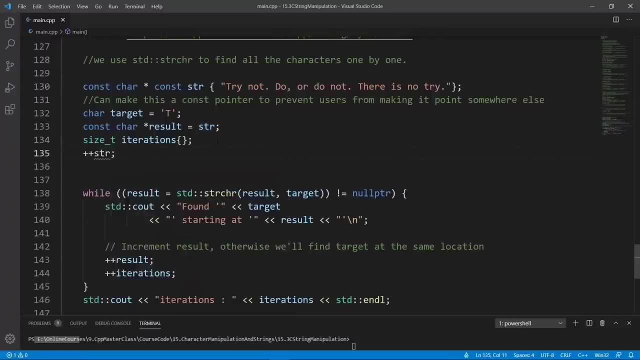 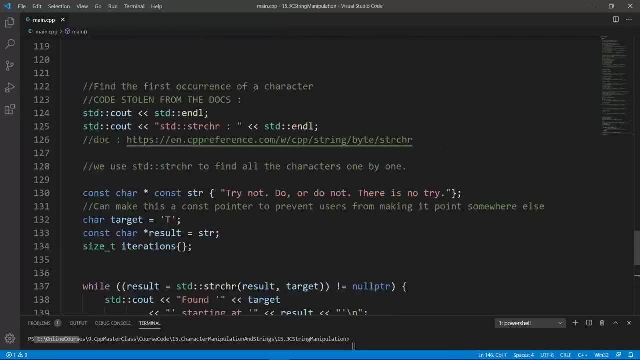 that, for example, we try and do plus plus htr, we're going to get a compiler error because this is a cost pointer by now and this is much safer. okay, we're going to comment this out and show you something that might throw off many of you guys. so we're going to comment this out and i am going to bring that in. 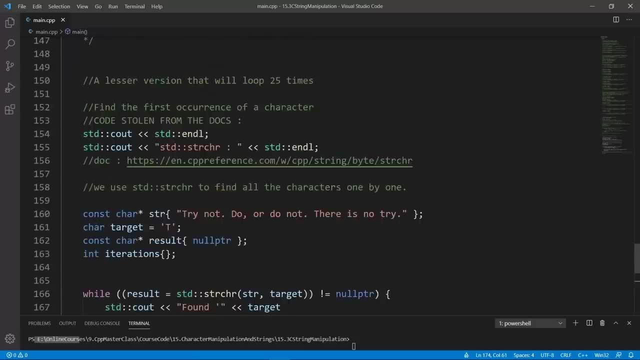 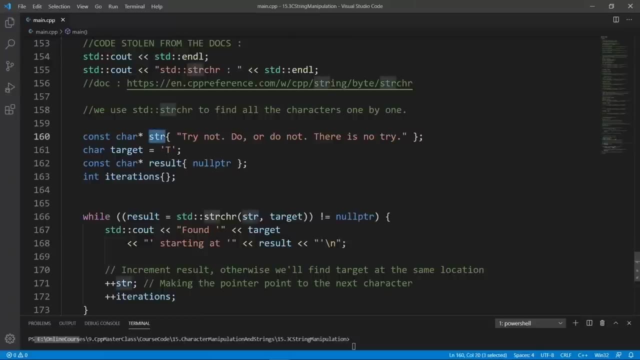 okay, let's go down here and we are going to do basically the same thing, but we will try and use htr in the first place here. okay, this is how we're going to do this. we're going to have our strength, we're going to have our target, we're going to have 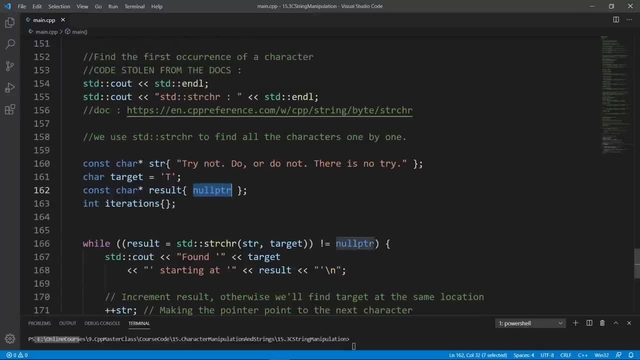 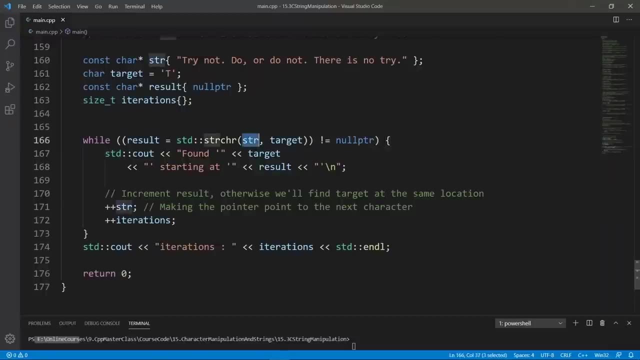 result here, which is equal to null pointer, and we have our iterations, which is an integer. let's make this a size t and what we're going to do in here: we're going to use str to search, okay, and we're going to basically do the same checks. we're going to jump in here and say: we found target starting. 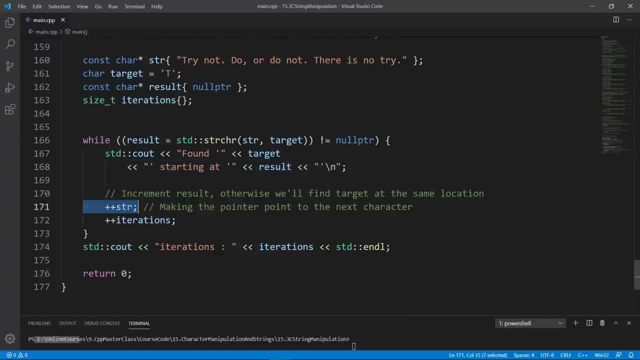 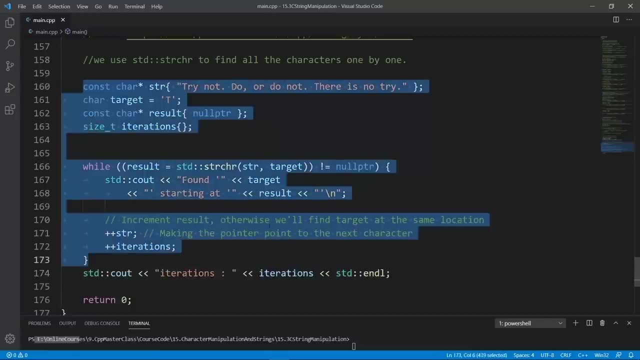 at result and we're going to increment str here because it is not a cost pointer. now, try to go through this thing here and see how many times you're going to loop. okay, go through it and when you are done, we're going to try and run this. we're going to build with gcc. the build is going to be. 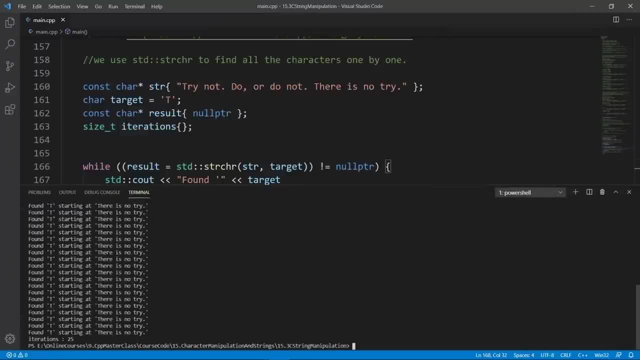 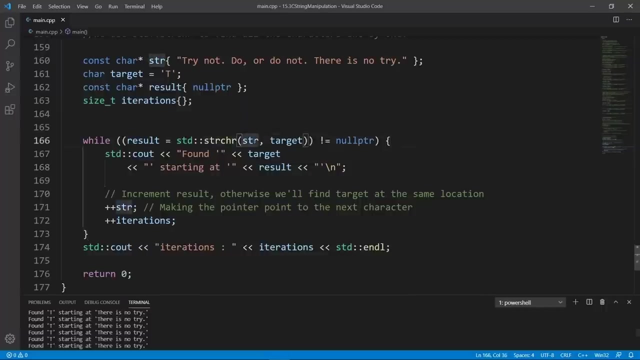 good, we are going to clear and run rooster and you see that this guy is going to loop 25 times and this is crazy. why is this happening? why is this happening? what we really are doing here? we are not assigning the result in the strength that we are searching at. okay, let's try and go through this a couple of times. so the first: 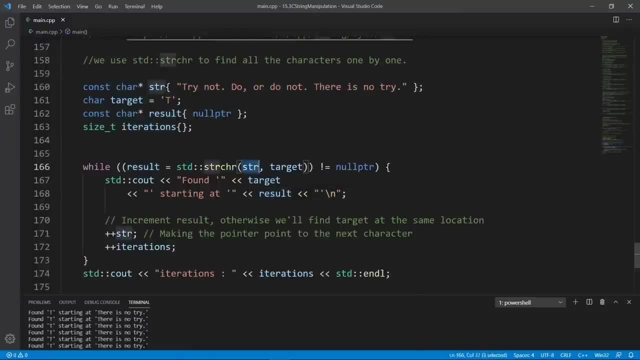 time we're going to do our search, okay. so we're going to search in str and if we find our target, we're going to return the pointer to the target. if we don't find it, we're going to return a null pointer. the first time we're going to find this t here, okay, and we're going to return a pointer. 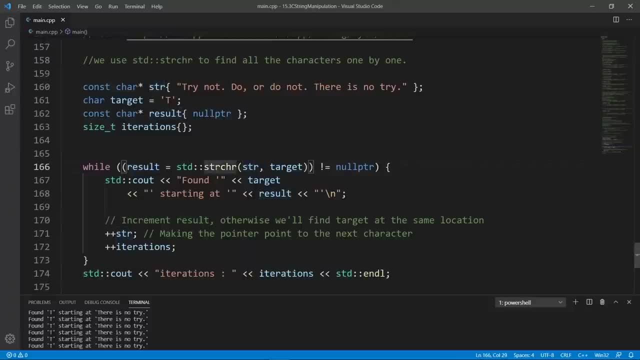 to it and store that in reserved, okay. so after we do this, we're going to fall in our body here and we're going to say: we found t starting at this location here. that's going to work and we're going to increment astr. okay, notice that we're not incrementing the result here if 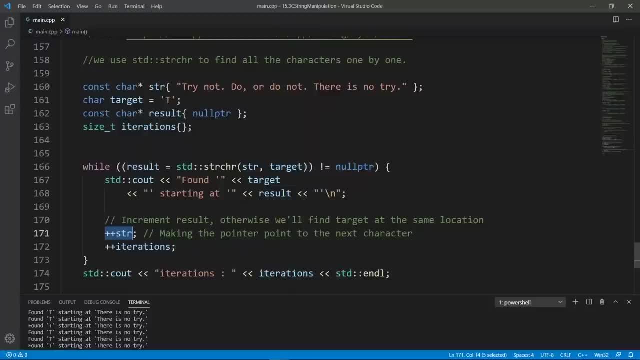 we increment str, it's going to point to the next character, which is r here. okay, and we're going to increment our iterations and we're going to start and loop again. we're going to search in here and we're going to be searching from this location here and we're going to find a t, starting at this. 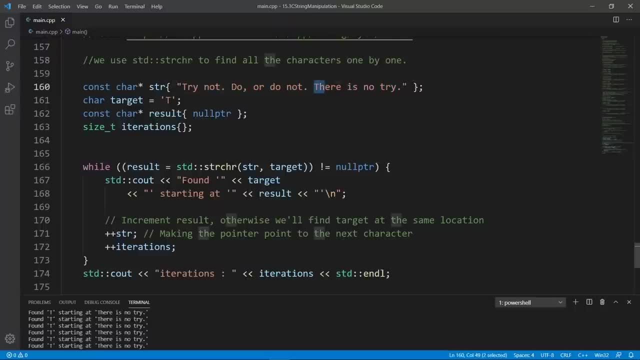 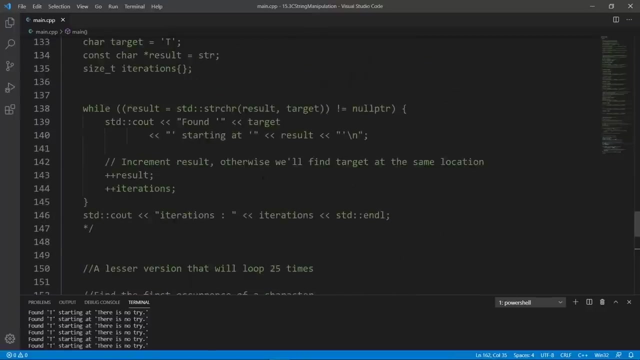 location. we are going to find this t here and we're going to return that and store that in reserve. but the problem is that what we are incrementing here, but the problem here is that we are incrementing one by one. we are not jumping to this t here and we had a way to jump to this t. 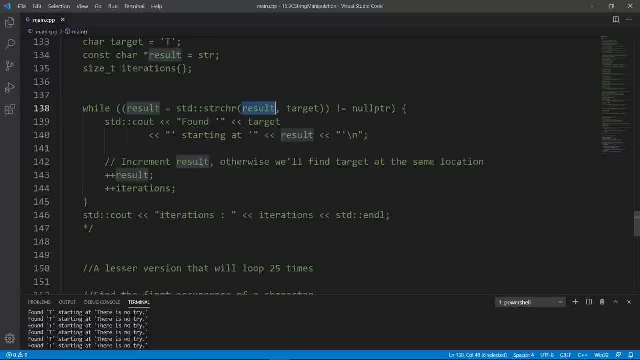 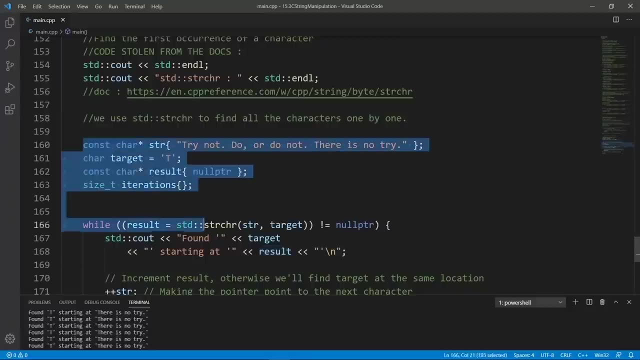 by assigning the result into the same variable that we are searching in. okay, so this is going to loop 25 times and it is not really good and some of you might try to set up something like this and it is really not going to be good. try to go through this and you're going. 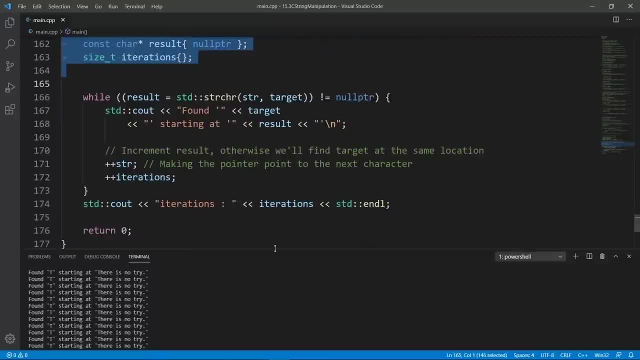 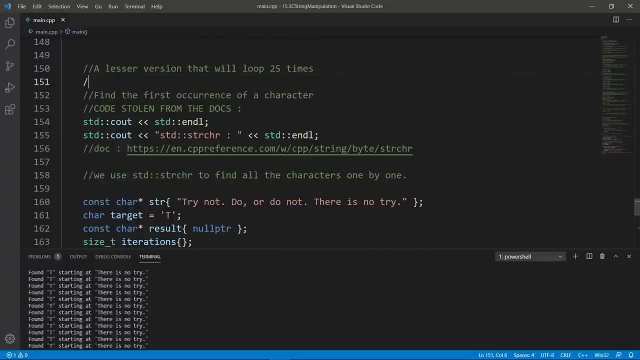 to see the reason why it is looping 25 times. okay, i wanted you to see this. don't do something like this- and we are going to comment this out. the next thing we're going to see is how we can find the last occurrence of the character, and this is a really cool example. i like it. it is going. 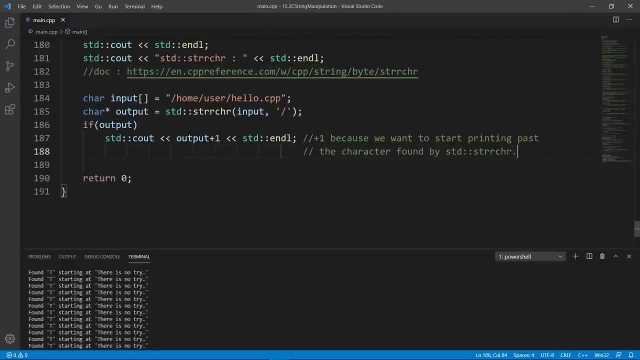 to do something very practical. we are going to take a path which is going to be an array, basically stored in this input array, and we're going to strip off all the things we don't need and we're going to hunt down for the file name from a full path, and this can be useful in. 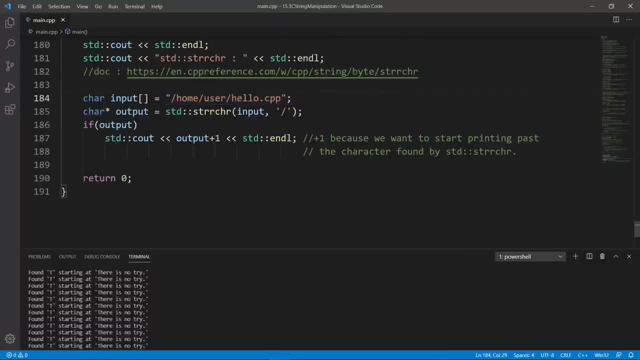 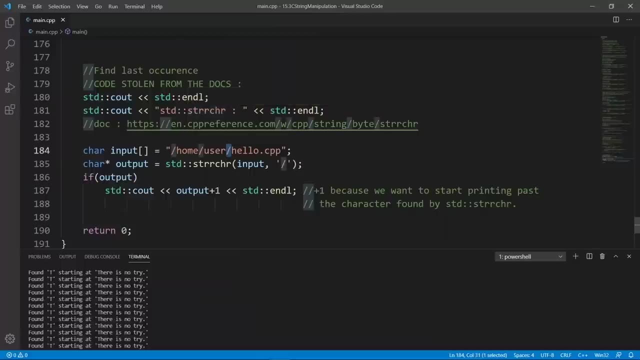 whatever application you are doing. so we are going to hunt for the last occurrence of a backslash character using the strr chr facility in the c++ standard library, and you can find the documentation on this guy here. i'm not going to go there. you should really practice to go there and read what. 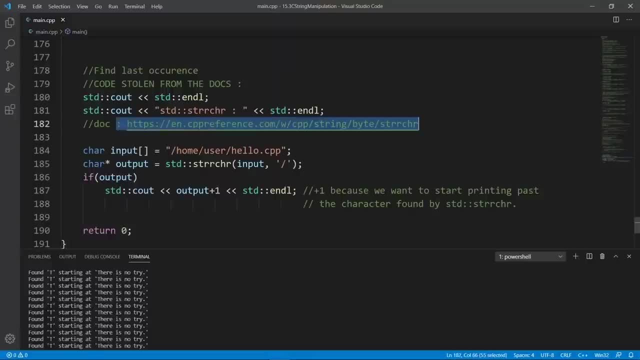 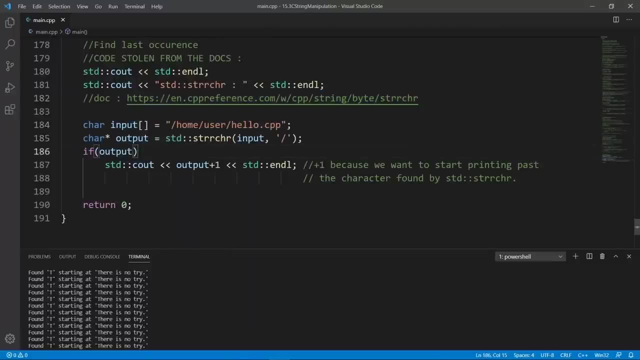 these things do. that's why i am leaving in the links to the documentation. you should go there and read and if you have a problem you can ask me. i will do the best i can to help you out. so this line here is going to hunt for the last backslash it's going to find. 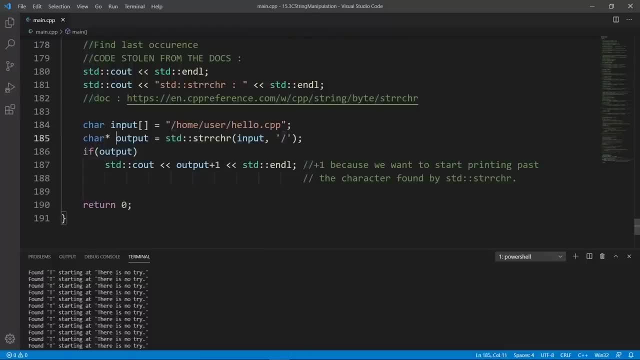 this guy here and we're going to store a pointer to that in our output character pointer here. after we do that, we're going to say if we found something useful, if this is not more pointer, we're going to print that out. but we don't want to print starting from the backslash. 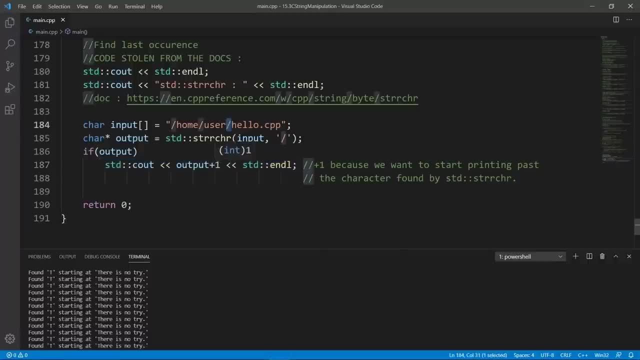 we are going to use pointer arithmetic and move to the next character, which is going to be this h here. so if we print this out, we're going to have hello cpp printed out, because stdc out is going to print until it meets the last null character and that's going to be. 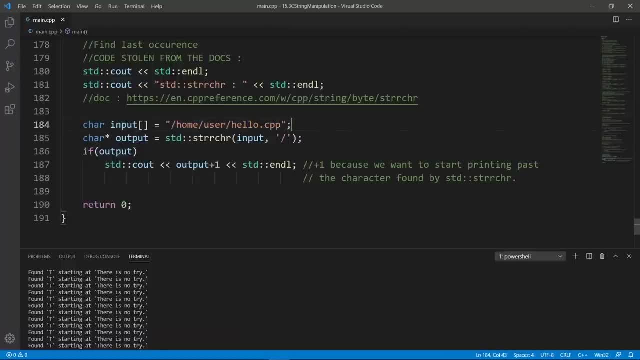 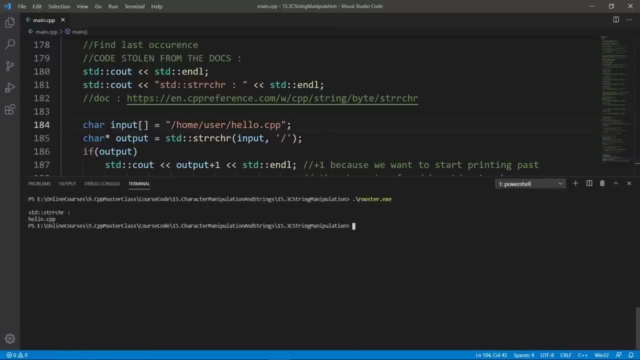 after the last p here, because this is a c string, literal here. okay, we're going to work this, the build is going to be good, we're going to clear and run rooster and you're going to see that we have hello cpp printed out here. okay, this is really all we said how to do in this lecture. 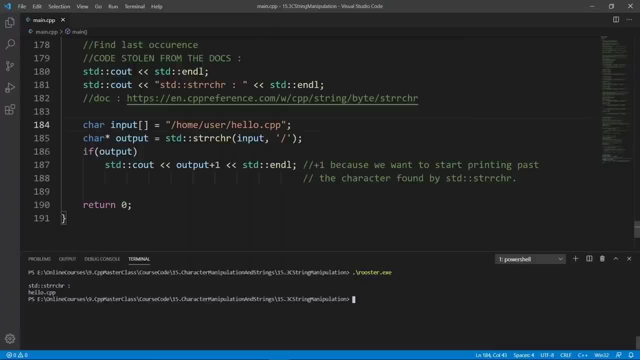 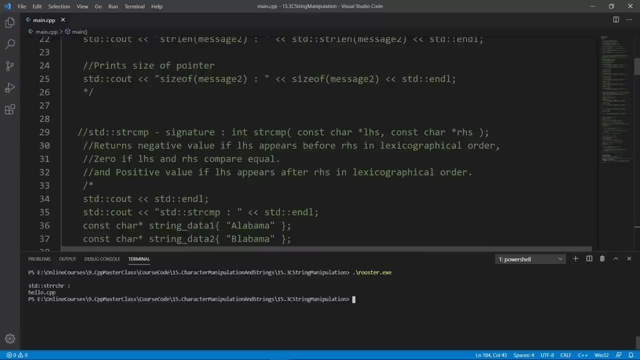 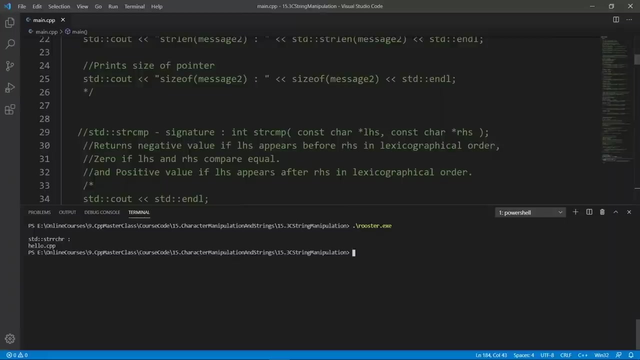 i apologize that it turned out to be lengthy. these things can take long to explain and i really wanted you guys to have as many explanations as i could come up with. we are going to stop here in this lecture. in the next one we're going to see how we can copy and concatenate c strings. 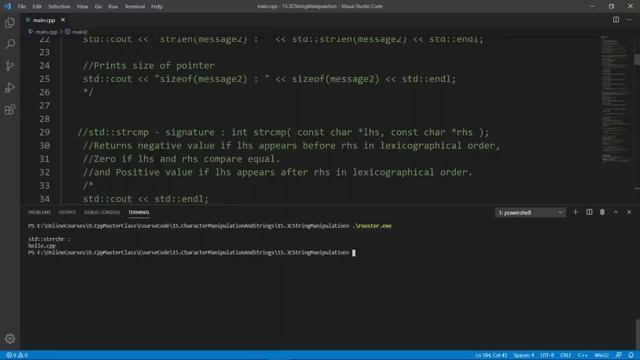 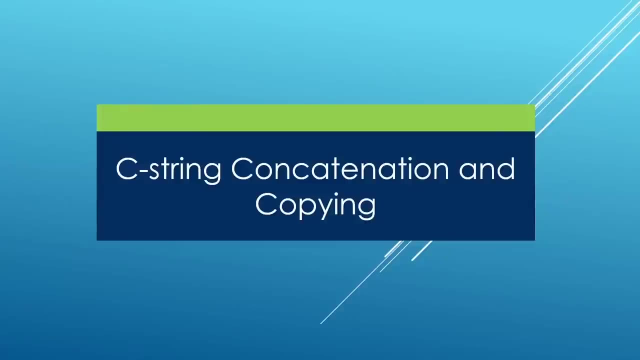 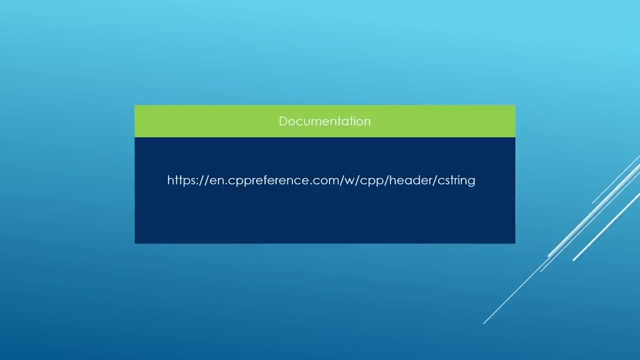 using the facilities from c string here. go ahead and finish up here and meet me there. in this lecture we're going to look at a few more facilities from the c string library and those are going to allow us to concatenate and copy strings over. the documentation for what we're going to be talking about can be found here. if you go there, you're going to fall. 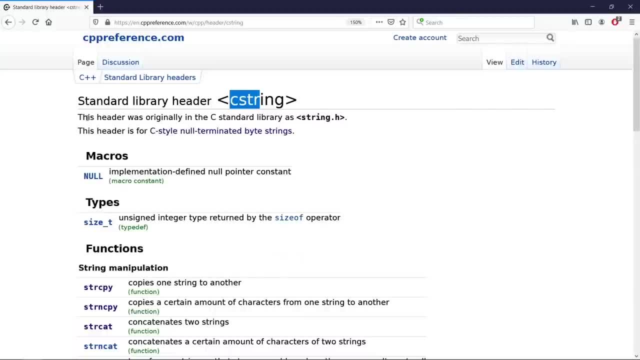 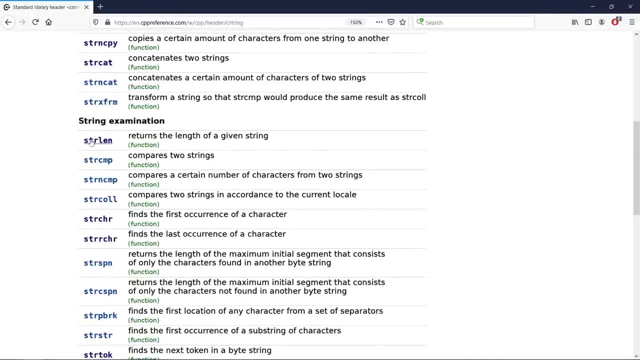 on this link here and you're going to find that c string was originally in the c standard library as string dot h, but in c plus plus we can use it like this. we have a couple of functions. we can copy stuff, we can concatenate, we can get the string length. we have seen this, but now 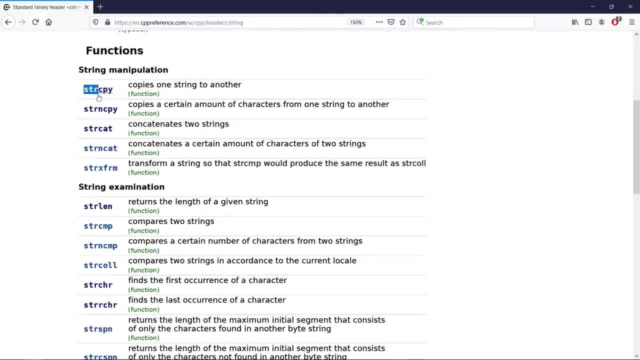 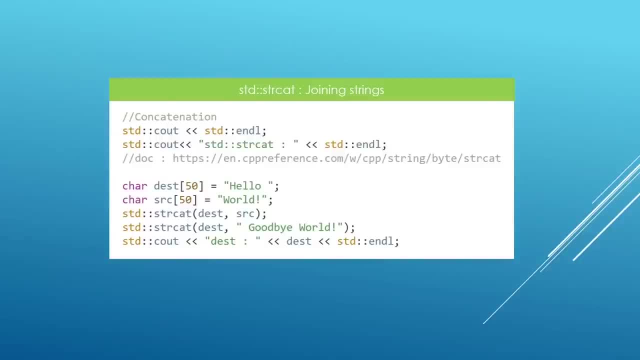 we're going to look at things that allow us to copy and concatenate stuff, because that's something you may want to do a lot. the first example we're going to look at is stdstr cat, which is going to allow you to join strings again. you can browse through the documentation here and see more about. 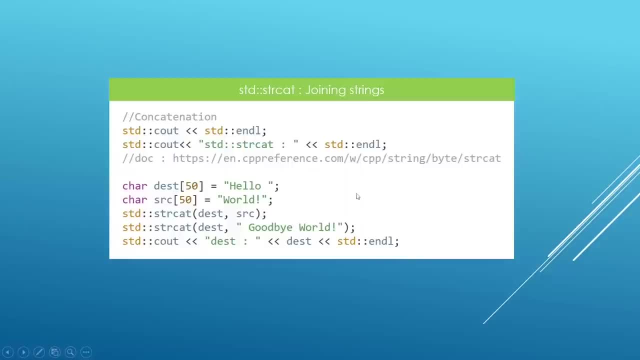 this facility here and you're going to see all about it. for now, we're just going to play with it. we're going to set up two arrays. one is going to be called dest. it's going to contain hello. the other is going to be source- here- and it's going to contain world. notice that these are row. 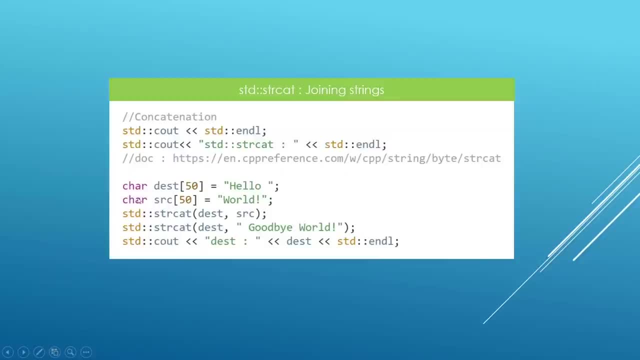 static arrays that are stored on the snack, and, uh, that's how we set them up here. okay, so we can concatenate strings using the syntax like this: we're going to say std, str, cat, we're going to say the destination string and we're going to say the source string we want to copy from. okay. 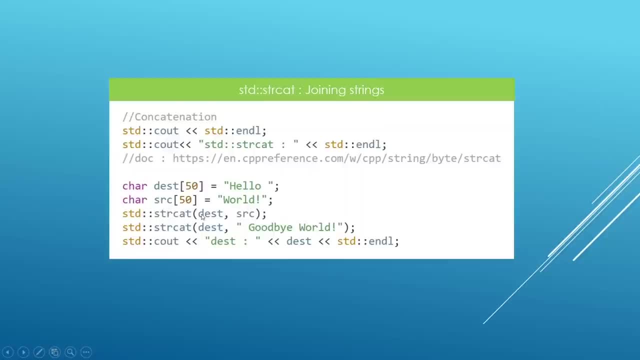 so after we do this, the destination is going to contain these two strings joined together. but before you do this, you have to be sure that your destination string is big enough. and this is a problem because you have to really keep track of your destination string and it is easy to put in many. 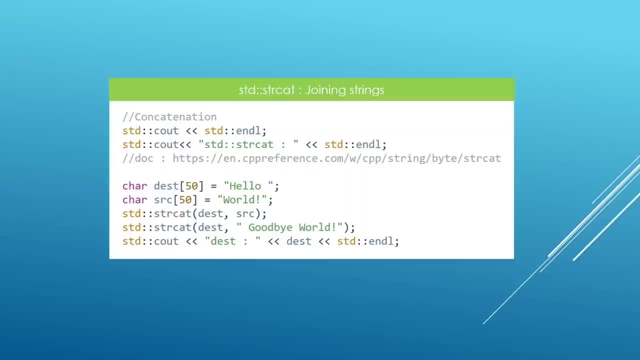 more characters that can really fit in the destination string. that's the reason many of this functions here are considered unsafe by many compilers. i don't think you can compile this on visual studio. it's going to stop you from doing this because of this way. have to keep track of things yourself, but i am just showing you so that you know how to avoid. 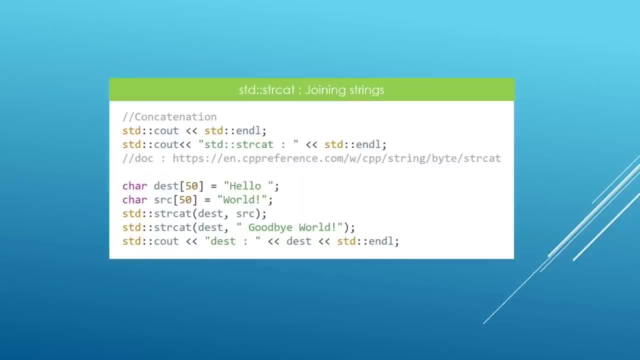 these problems if you happen to be on a compiler that doesn't protect you from this. so we're going to append goodbye world to whatever is in dest and down here. if we print dest, we're going to have hello world, goodbye world, printed out. we are going to play with this in a visual studio code, in a 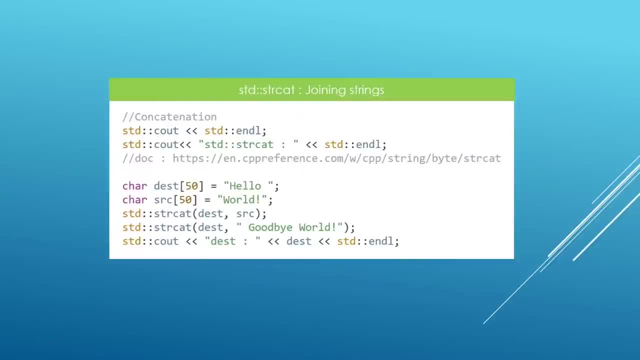 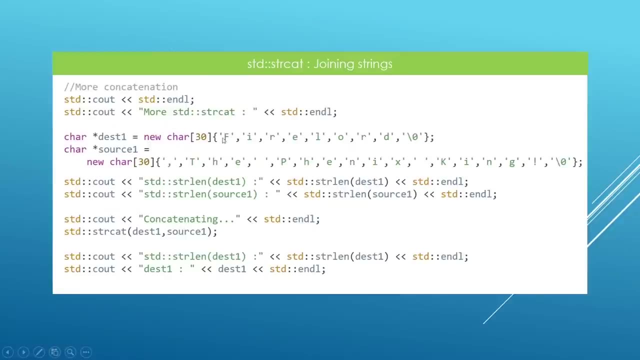 minute. don't worry if any of this doesn't make sense. yet here is another example of how we can join strengths through str cat. we have two strengths and we set them up with a simple characters like this. you can do this and put in your own null terminating character. this is a 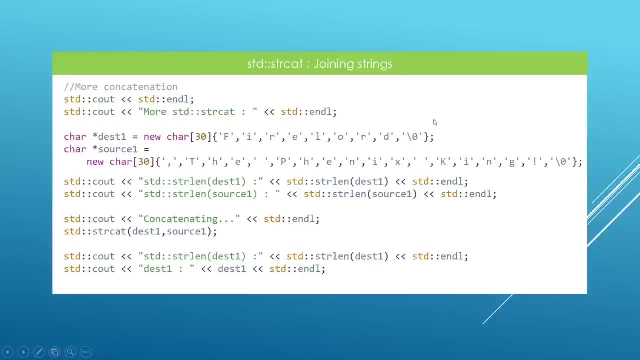 legal c++ code and notice that this array is a dynamic array. it's going to live on the heap because of this new operator. here we also have a source array which is also going to live on the heap. it is 30 characters long, so it is really long and we're going to try and concatenate. 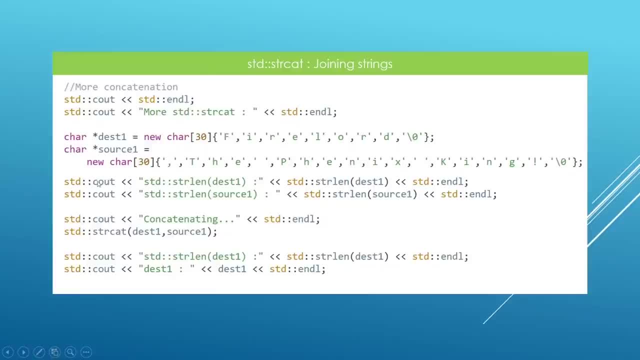 this with a string and we're going to try and concatenate this with a string and we're going to check their lengths, we're going to print them out and we are going to concatenate. the syntax is the same. you are going to say str- cat. you're going to specify your destination and your source. you're. 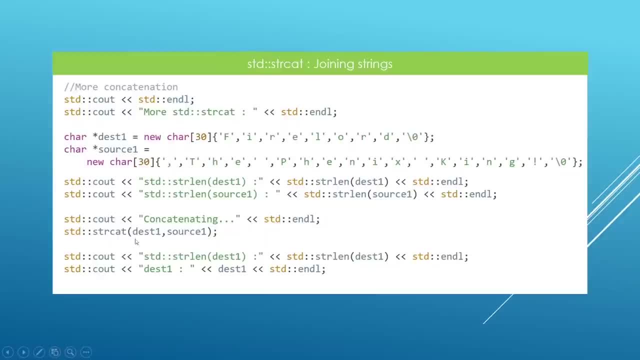 going to be copying stuff from and you are going to store the result in destination here. what this is going to do, it's going to grab whatever is in source and copy it. so it's going to copy the entire thing here from source and it's going to append that to whatever we have in destination. 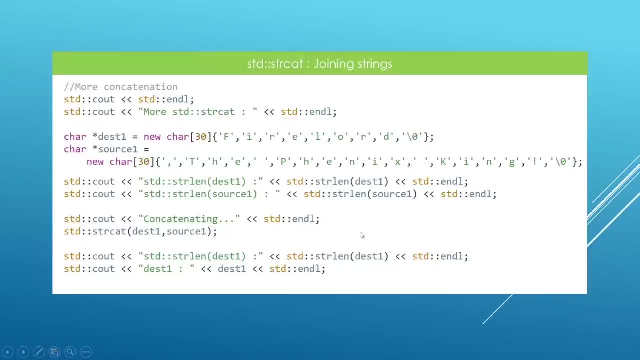 starting from the last null character here. so it's going to overwrite from this null character and it's going to basically copy everything in the destination here. and if we print whatever we have in destination here, we're going to have fire lord the phoenix king printed out and you're 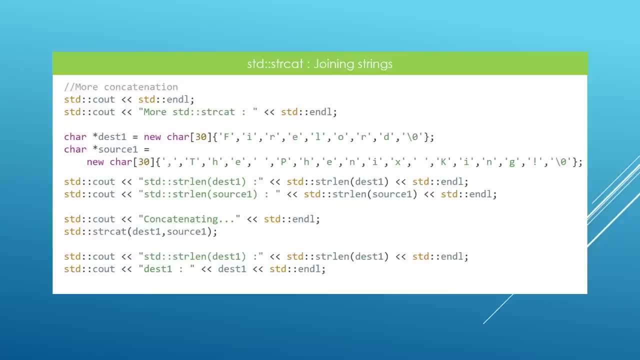 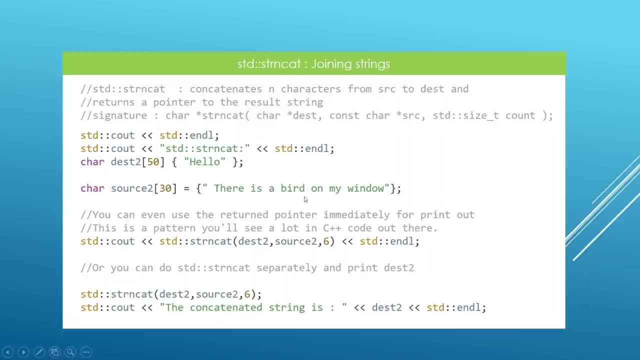 going to see that this is going to be the case when we hit visual studio code in a minute. you can also use a version of the str cat version that is going to allow you to specify how many characters you want to concatenate from the source string. in this case, we have destination. 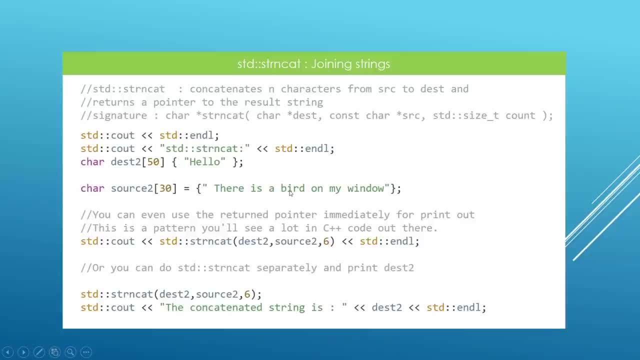 which is hello, and we have source, which is there is a bird on my window and down here. you see that we do str in cat. we say the destination, we say the source and we say how many characters we want copied from the source here and we say six characters. so we are going to count from the 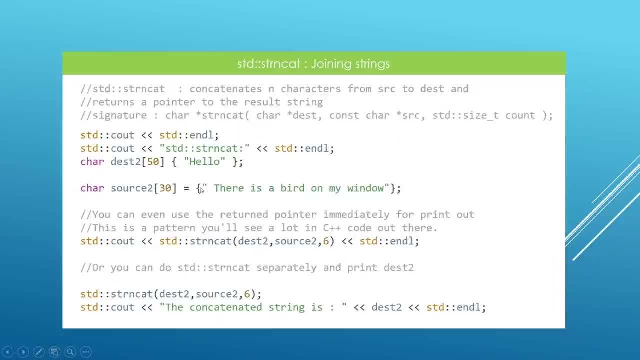 source. we're going to say: one, two, three, four, five, six, we're going to grab this there, string with this space here, and we're going to append that to the source and that's what we're going to get in here. we're going to say, hello, space and there, and that's what we're going to. 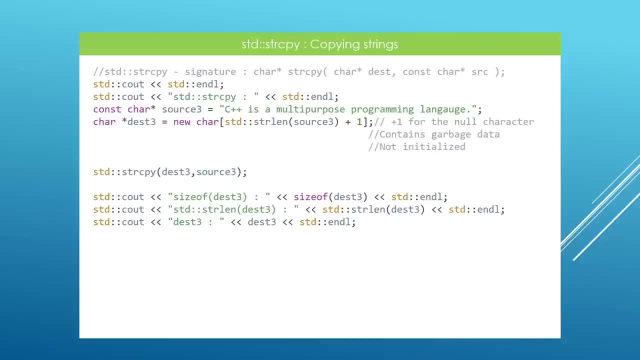 have printed out here. if we print dest, we can also copy stuff, and the str cpy function here is going to do that, and here we have an example that is going to try and drive this home for you. we have a source string which is c plus. plus is a multi-purpose programming language. okay, dest. 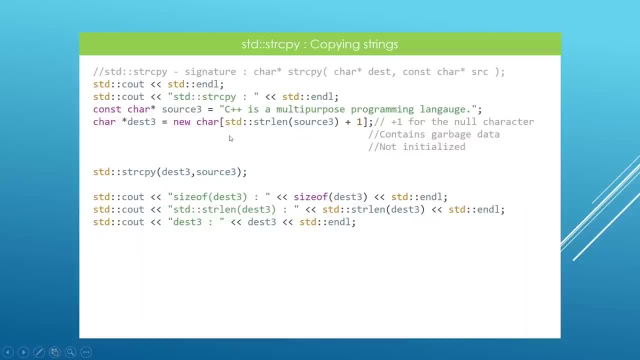 here is going to be the same length as source. we made sure of that in here because we're going to grab the length of the source string. please remember that str len is not going to count the null character. that's why we are adding a one here to account for the null. terminating. 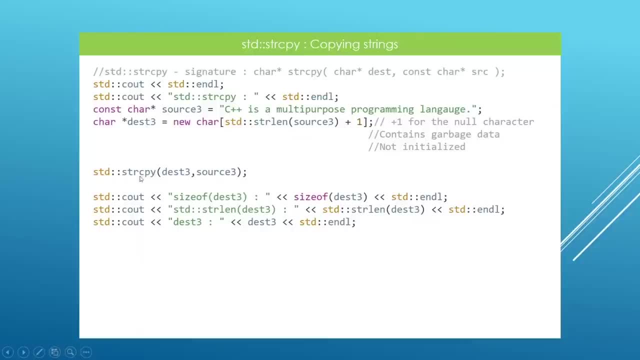 character here. okay, after that we're going to jump down here and say str cpy, dest three and source three. we are basically going to be copying from source and pasting in destination here. that's what we are doing. if we print destination, we're going to see that now it's. 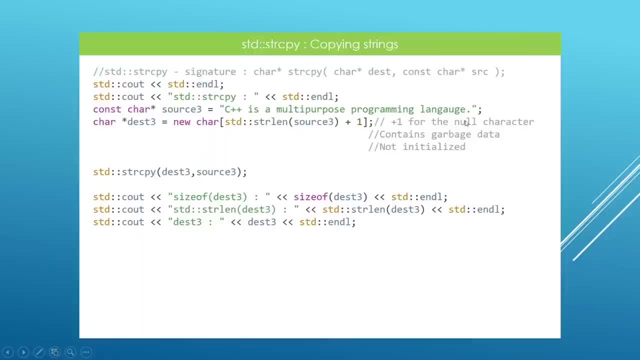 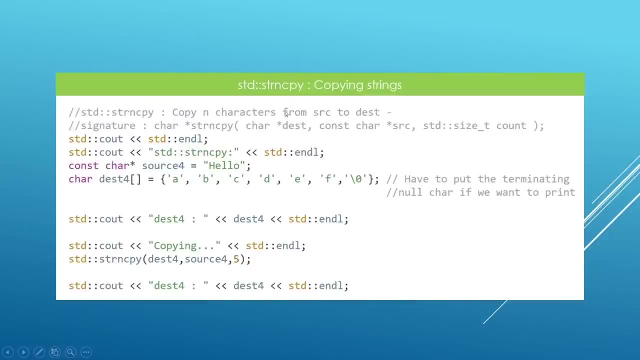 going to contain whatever we had in source, and this is how you can use these methods here. we also have a version with which we can specify how many characters we want copied from the source. here we have a source string which is hello. we have a destination string which is dest four. 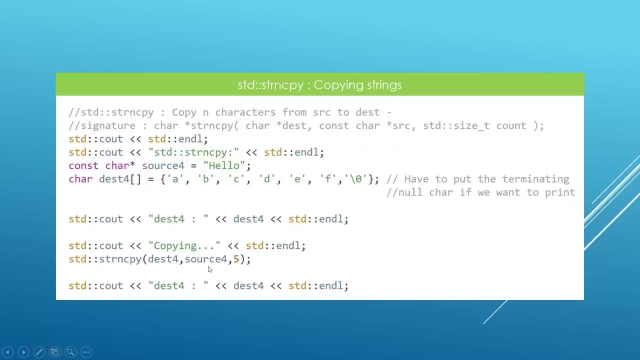 and we are going to copy stuff. we're going to copy from the source, we're going to paste in the destination and we are just going to copy five characters. what this is going to do is copy everything from the source and paste in our destination, and it is going to override whatever we have in the starting indexes in. 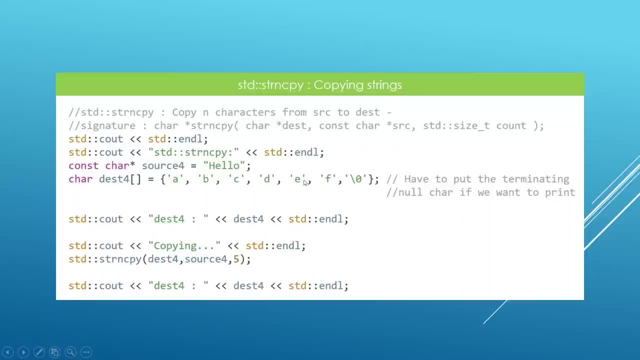 destination here. so we're going to have a, b, c, d, e here replaced by hello, and if we print dest here, we're going to have hello f printed out. this is how these things work, and if you wonder how i know how these things work, i just come and read the documentation. 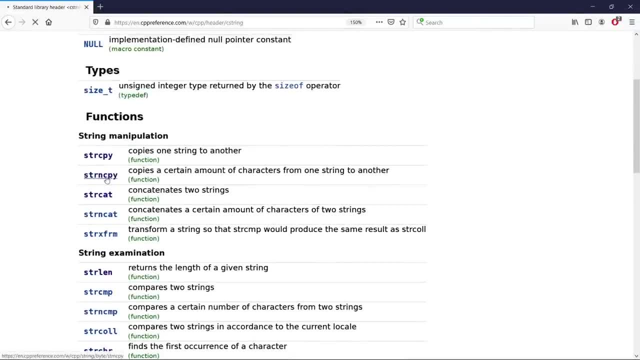 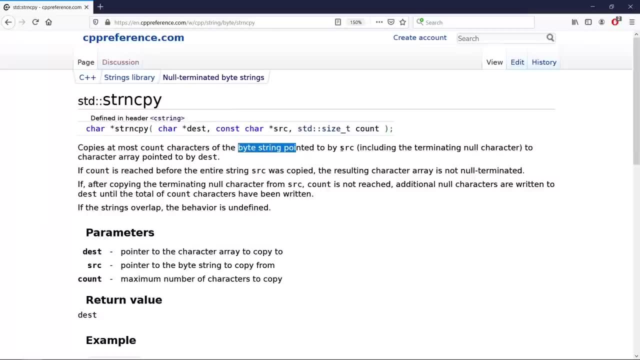 here, for example, hdr and cpy here. if we click on that we are going to get the documentation. this is going to say copies at must count characters of the byte string source, including the null terminating character to the character array pointed to by dest. that's what it does, we. 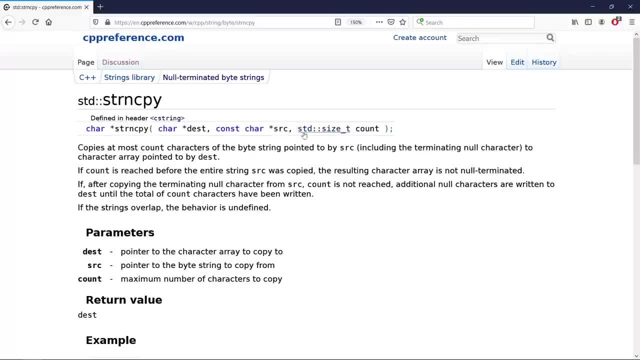 have the destination, we have the source and we have how many characters we want copied, and they say a few things. you need to be careful about this guy here. one thing that you usually care about is the return value. you see that the return value is going to be the destination string. so if you want this pointer, you can use it and you 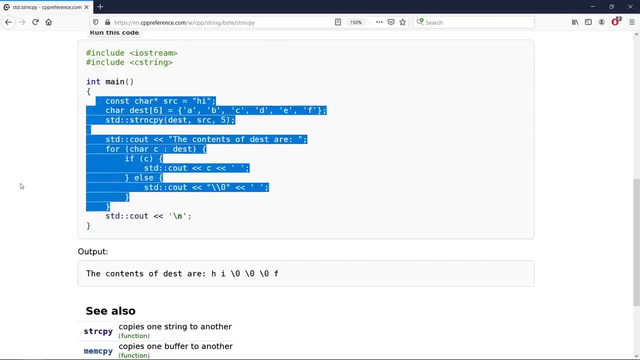 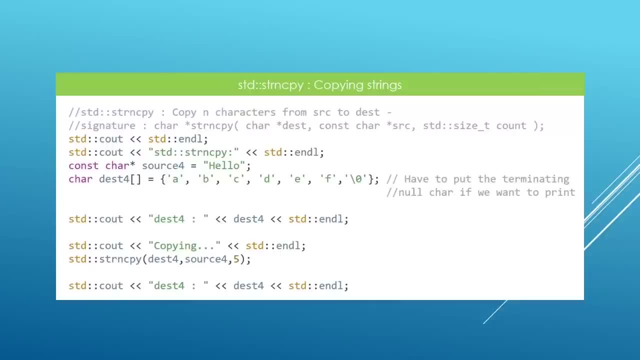 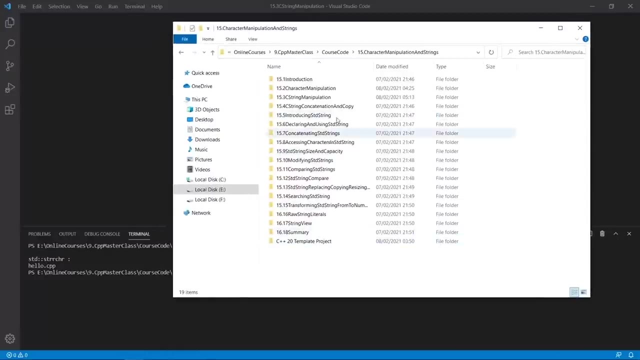 can go down and look at a few examples here and play with them to really drive the point home. okay, now that you have an idea about how these guys work, we are going to head over to visual studio code and play with them right away. okay, here we are in our working folder, the current 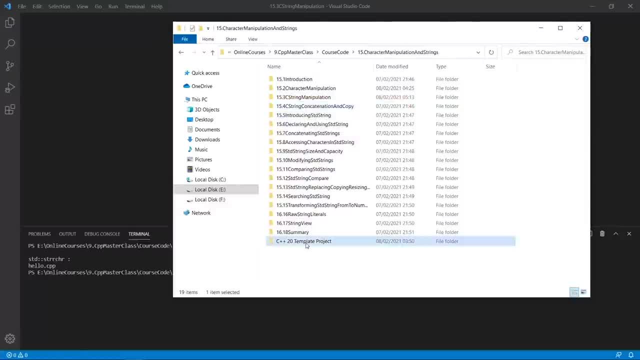 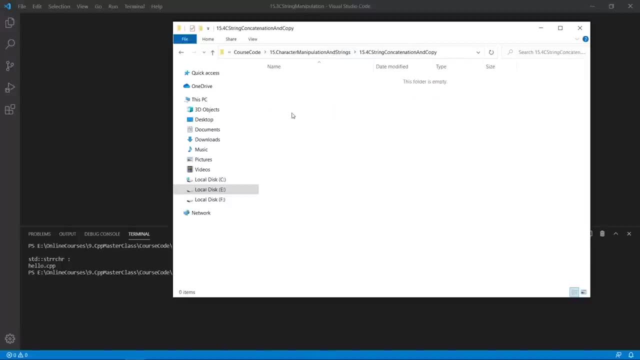 project is c string, concatenation and copy. that's what we are doing here. we're going to copy our template for our c string and copy it. we're going to copy our template for our c string and copy it files and jump to our current project and put them in place. we're going to open this in visual. 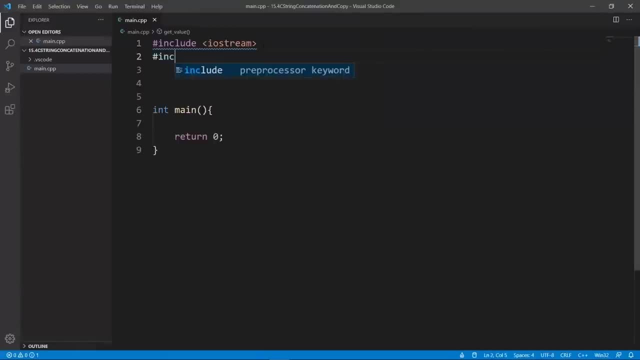 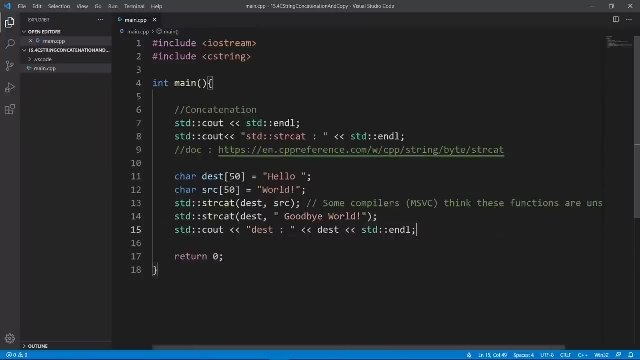 studio code pretty quick. we are going to include c string because that's what we're going to be using here. we are going to bring this up a little bit and we are going to put in our first example. here we have two strings, destination and source, and you see that we tried and made sure that they 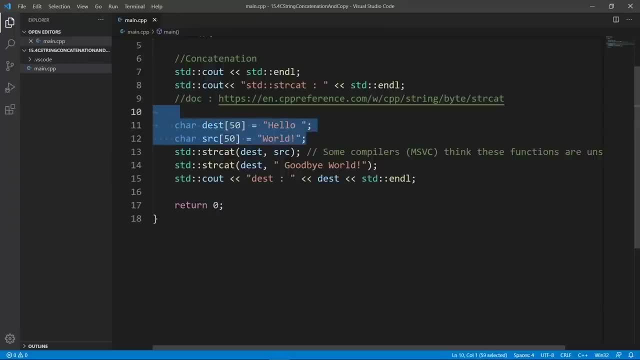 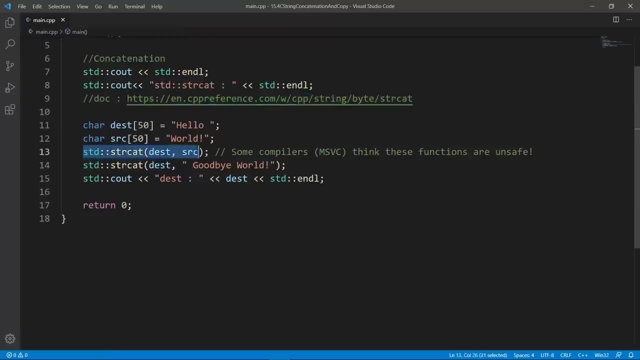 are large enough to contain however many characters we want to put in and they are row arrays stored on the stack, because they are set up like this and again, you can check out the documentation here if you want to know how this function works. and we are going to call str cat. 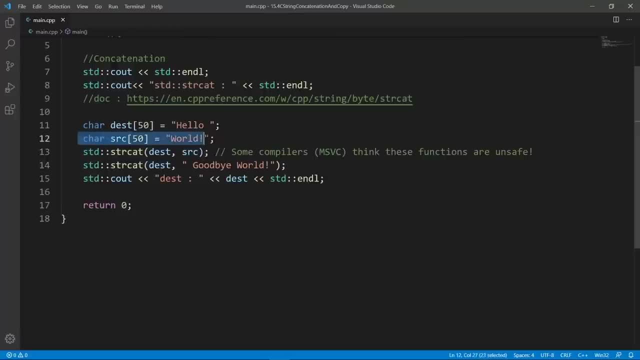 here to concatenate the source to our destination here. so if we do this, we're going to have world here concatenated to what we have in hello here, and we're going to have hello world in place, for example, if we try and print this out. we're going to try and do that. 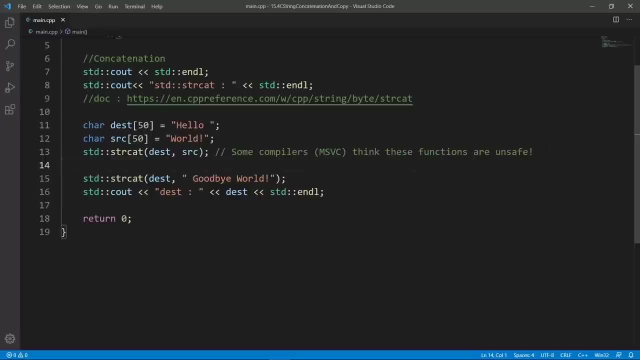 after we do the first concatenation here, let's do that. that's going to be better to show you how these things work. okay, after the first function here runs, we're going to have source concatenated to destination here, so what we're going to have is hello world stored in. 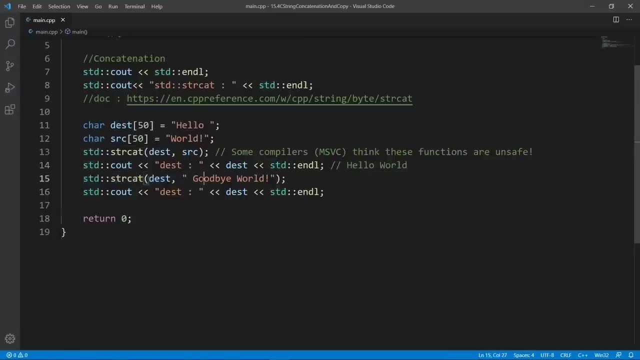 destination here. the second concatenation here is going to append goodbye world to whatever we have in our destination here. so we're going to have hello world stored in destination here. so what we're going to have printed out is- if we print that, of course, is hello world and goodbye. 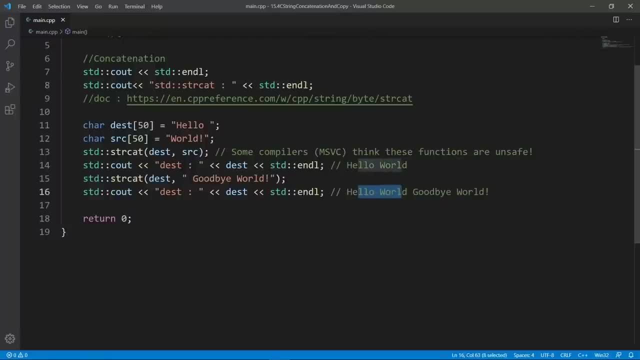 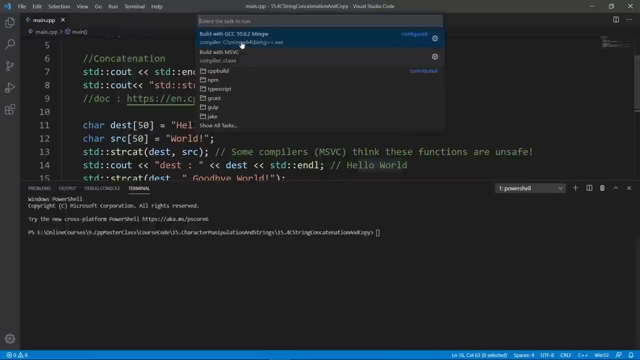 world. okay, we're going to have this writing down. let's try and run this and actually make sure that that's the case, and then we're going to see how this function can be unsafe for some compilers. we're going to build this with gcc. you see that it's going to go through, and if we run this, we're. 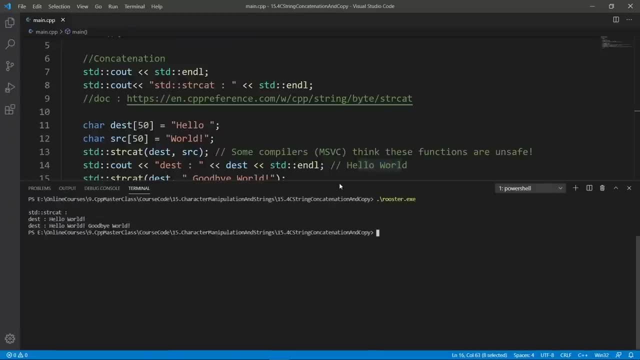 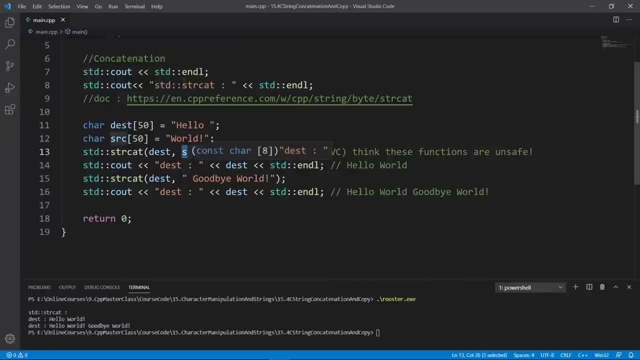 going to have hello world, hello world, goodbye world. printed out. this is what we expect and again, this function here str cat is going to have whatever you have in source and it is going to append that to whatever you have in destination. and for this to work, you have to be sure that. 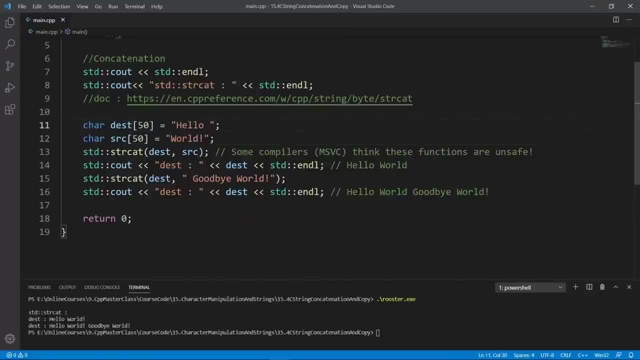 the destination is modifiable, for example, if it was an array of const car, let's do that and show you the compiler error. we should get a compiler error because now destination is not modifiable, it is an array of const characters and we can't modify it. so be sure. 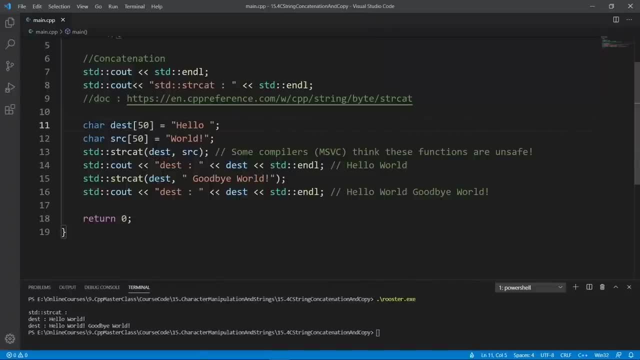 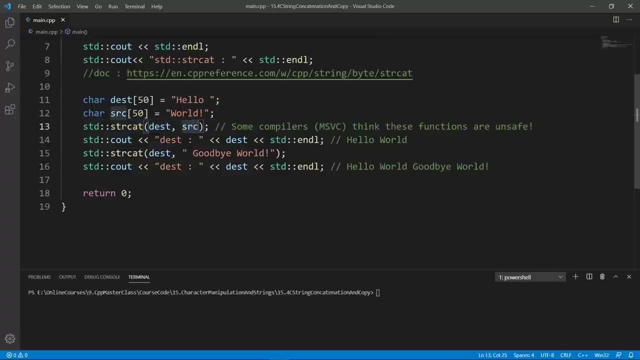 the destination array is modifiable and in this case it is okay. please know that some of these functions can be treated as unsafe by some compilers, but i tried this out on both on gcc and the compiler from microsoft and they work pretty well. so you can try them out here to prove. 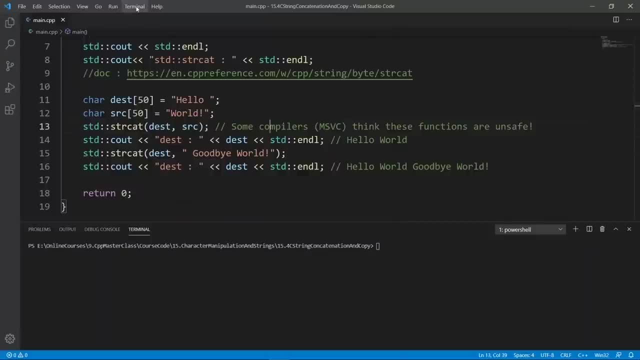 that let's go and try and build with the compiler from microsoft. we have it set up here. so we're going to run the task to build with msvc here and you're going to see that the world is going to be good. the build finished successfully and if we go in we're going to clear and run. 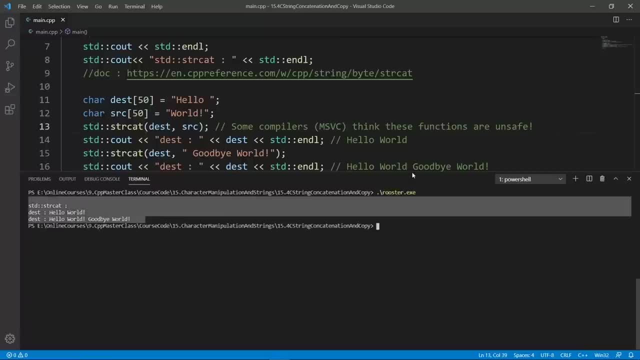 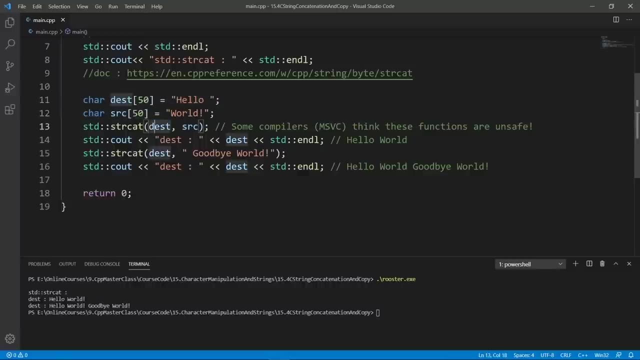 rooster, you're going to see that it is going to do exactly the same thing, but some compilers might give you warnings or errors if you try to do something like this. and the reason is you really have to be careful using these functions because if, for example, destination array is not large, 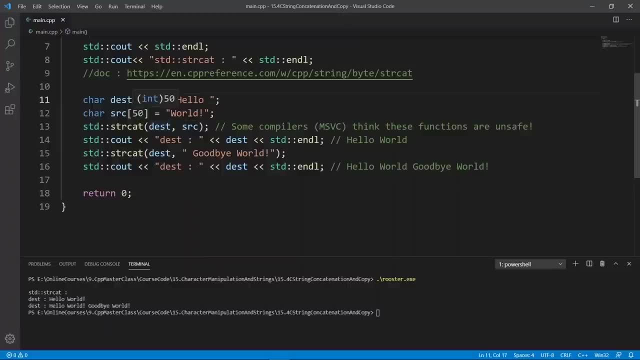 enough. you may do some crazy things running over the balance of your array and it can be really bad. for example, if we try and make the destination array not large enough, we're going to see that destination array here, for example, a size of three. it is possible to do that and you see that. 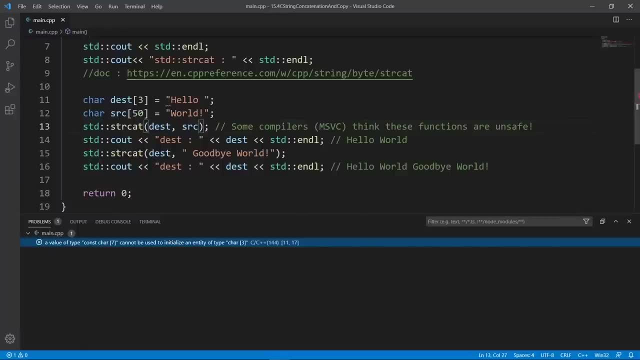 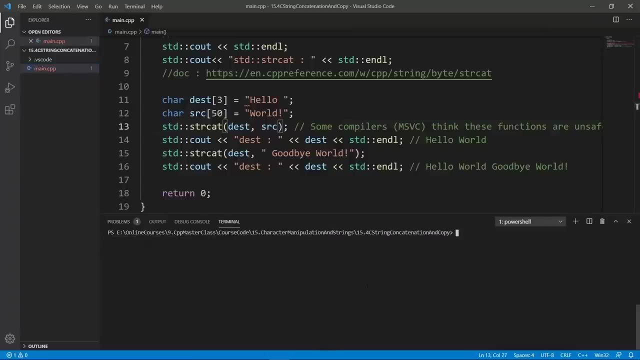 we get a warning from visual studio code and if we try and build this with gcc, let's try and remove the garbage we have from visual studio first. now that this is clean, we can try and build with gcc. let's do that, our compiler. we're going to choose gcc and you're going to see that it's going to. 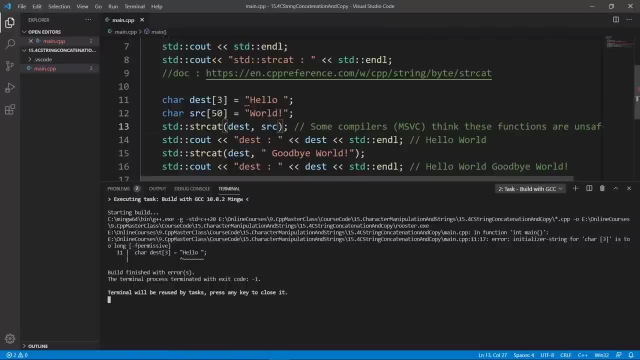 give you an error. it's going to actually protect us from doing something like this, but in some cases, some compilers are not going to stop you from doing this, but any compiler that really respects itself is going to have these safety checks in and it's going to protect you. 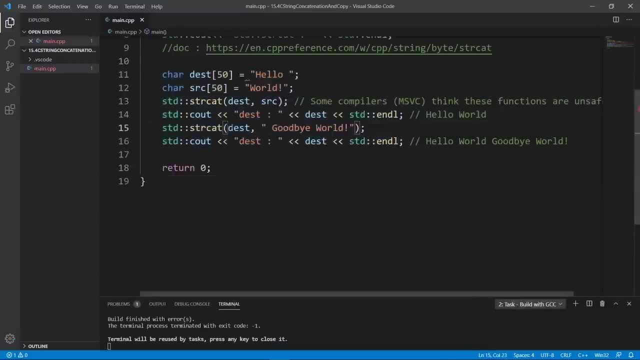 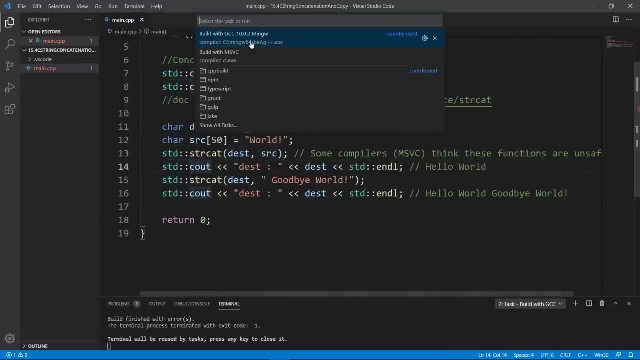 from doing something crazy like this. okay, this is how you can do concatenation using str cat, like we did here. let's try and build and see that now we are building fine, because i don't like these red lines here. the build is good and we are all fine. now i am going to comment this out. 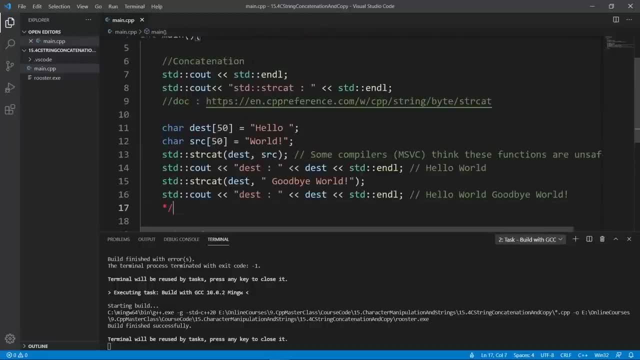 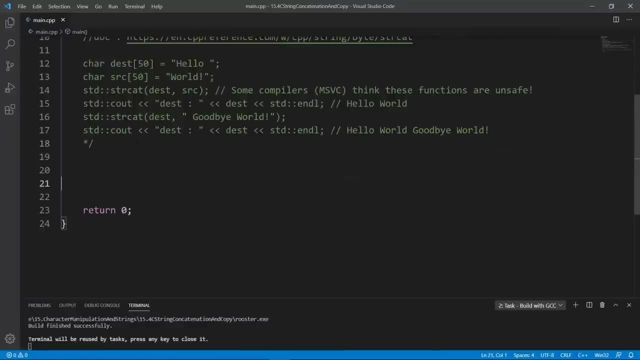 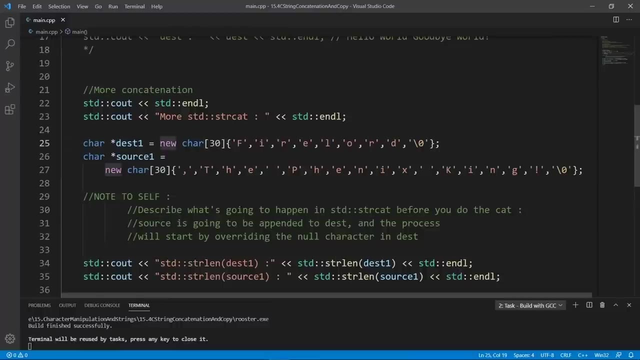 and we're going to see another example of how we can concatenate stuff. we are going to go down here- let's bring this down and hide this- and we are going to put in our simple example exactly the same thing we saw in the slides. we have two character arrays. they are dynamic arrays, but 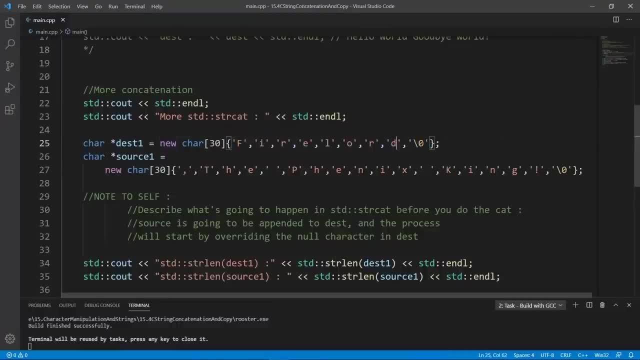 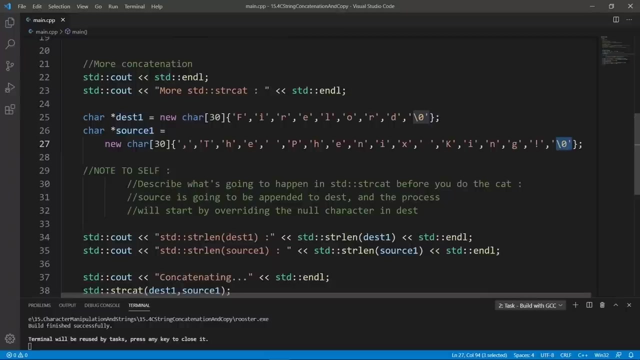 we initialize them with characters like this and we make sure to put in our null terminator. we have our source string which is going to say the phoenix king and it's going to have a terminator here. and what we're going to do, we're going to take source and concatenate that. 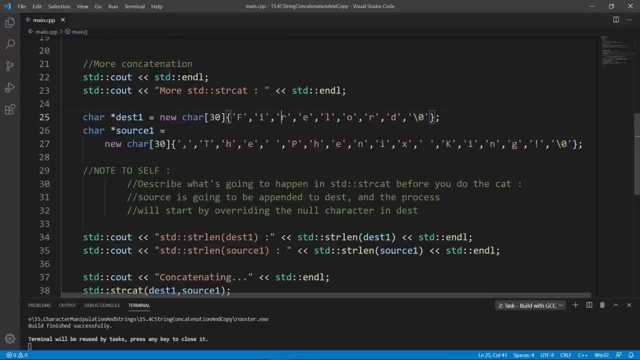 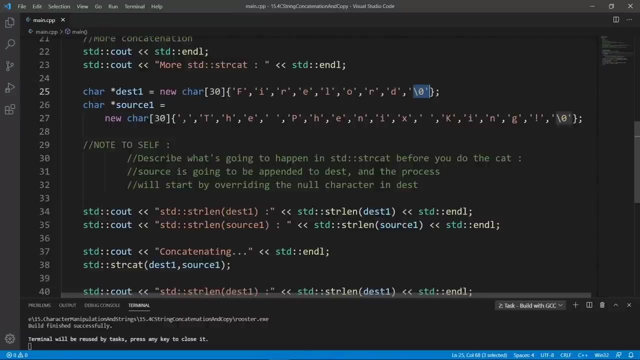 to our destination. so what is really going to happen? we are going to overwrite the null terminator here and we're going to start pasting in things from source here. so after the concatenation is done, what we are doing here, we are concatenating source one to dest one. we are going to have 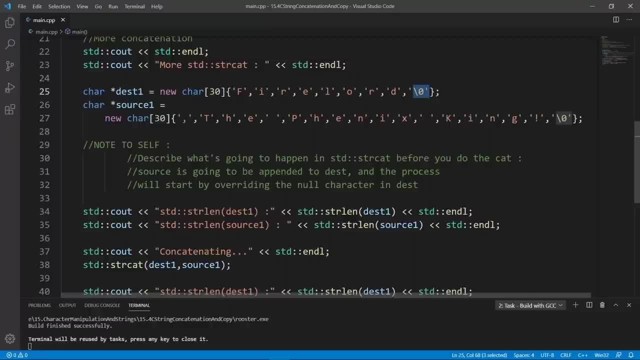 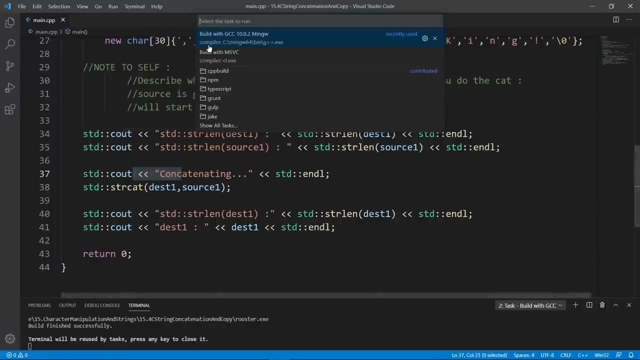 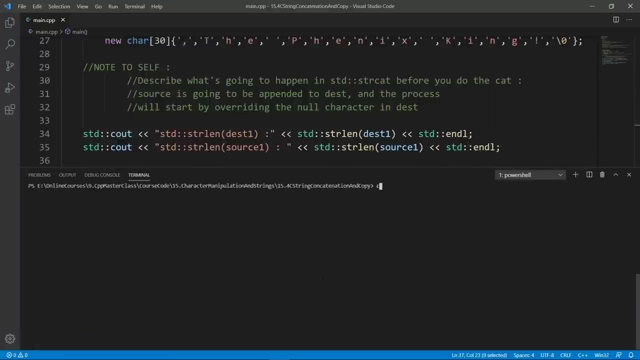 fire lord, the phoenix king stored in our destination string here we place the todosコンポ barn Here. So you can see we are wound on info right from car where we found the rest of our Ellis is so daemone and new only. 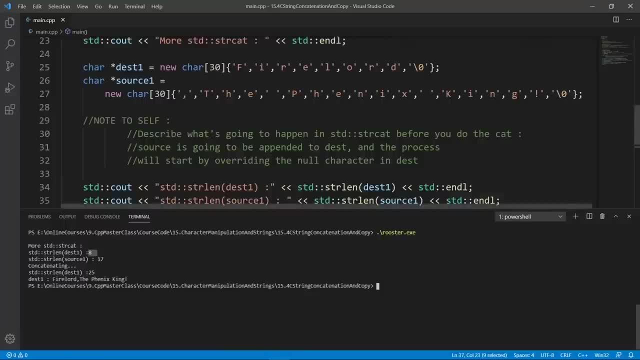 this new elise is going to. they can have signating information, delete, actually edit their settings. we are going to run this a. ok, let's go ahead and check this out. we're going to talk about it later. yet the group that we made sure that at least large enough to contain our characters here and if we print it out, the kinda thing printed out, we can try. 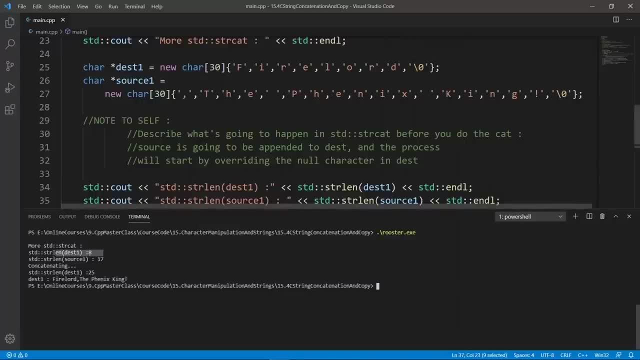 seven, eight- remember, strlan doesn't count the null characters, so this is what we expect: eight characters. the source is going to be 17 characters. if you count all this, that's what you're going to get, and if we concatenate them now, destination is going to be 25 characters long. in the eyes of 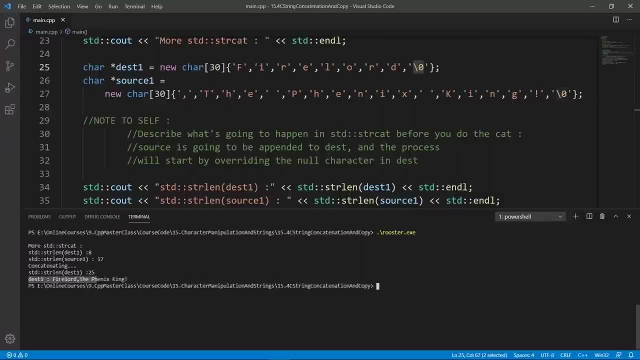 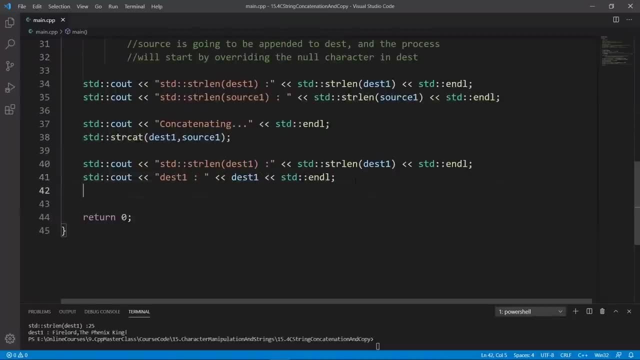 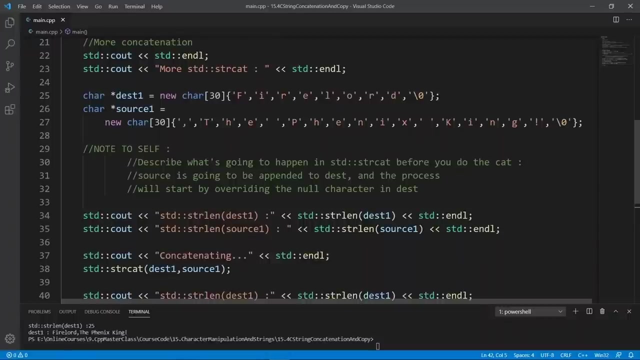 strlan and you see that we print the destination and it is exactly what we expect. fire lord the phoenix gang. okay, we're going to comment this out. i just wanted you to see an example of this, and the one thing i really want to stress in this example is that str cat is going to start. 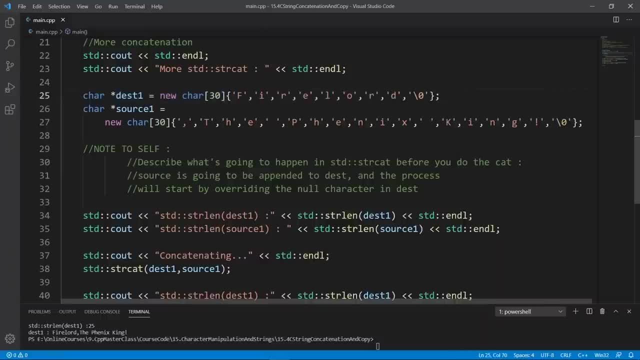 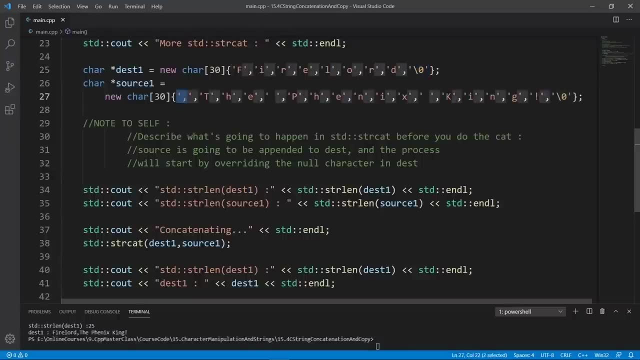 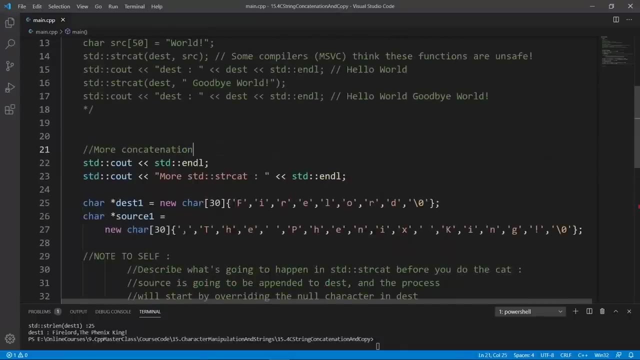 overriding whatever is in dest, starting at the last null character. okay, so this guy is going to be overridden by the comma here and we're going to start and put in stuff, and that's what we're going to see here. let's comment this out because we want to move on and show you a few other. 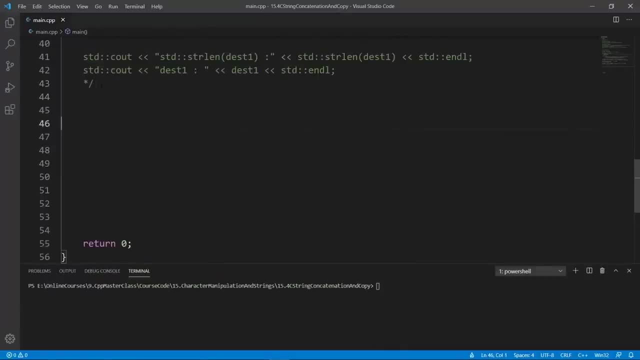 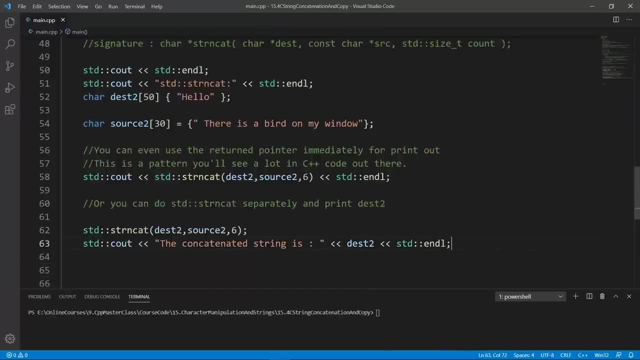 examples. okay, the next thing we're going to look at is a new version of str cat that allows you to specify how many characters you want concatenated from source. for example, here we have two strengths- destination and source- and here we are basically saying: i want to concatenate six characters from. 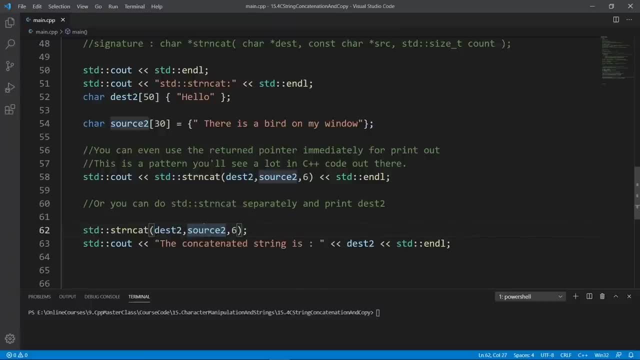 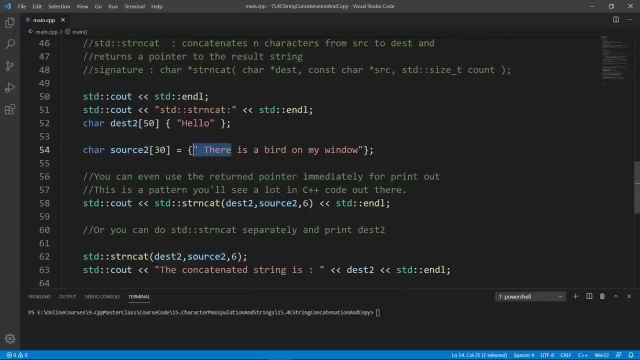 source and put them at the end of the destination here. and what it's going to do? it's going to grab one, two, three, four, five, six. it's going to grab this entire thing and it's going to append that to hello and we're going to. 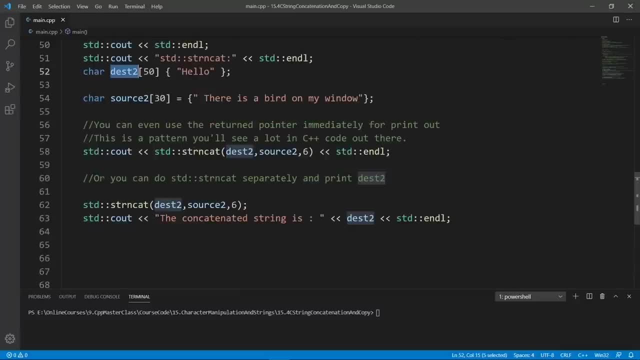 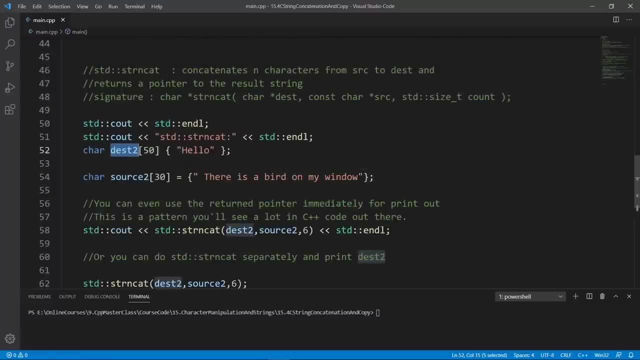 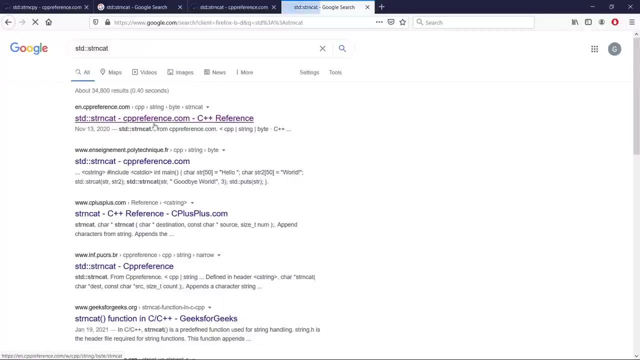 have hello there stored in the destination and the return value is going to be a pointer to destination two. and how do i know the return value? well, i know that from the documentation. if you go in your favorite search engine and do std, str and cat and you're going to see a link. 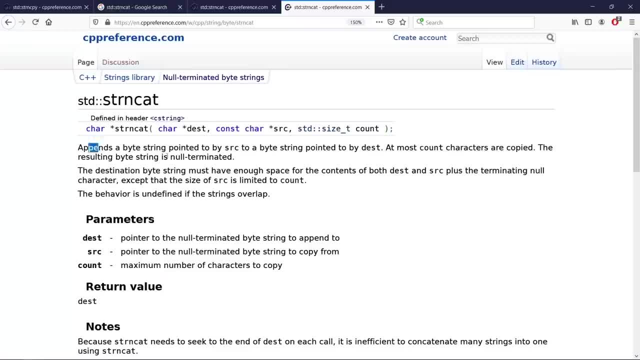 here. if you click on it from cpp reference, it's going to give you everything you need to know about this function. here it's going to append source to destination and n count characters are going to be copied. so the third parameter here is going to be how many characters you want copied and pasted into our 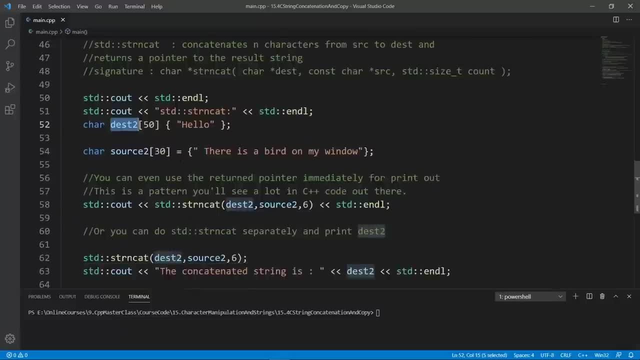 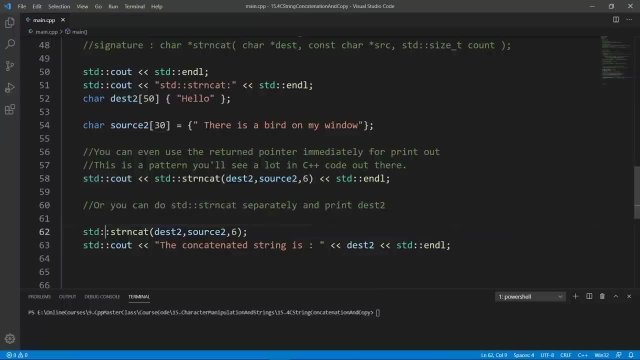 destination and the return value is going to be dust. okay, if we try this out, we're going to see hello there printed out. we're going to print it out directly and we're going to print that out using the destination pointer that is going to be returned from this guy here. so if we try and 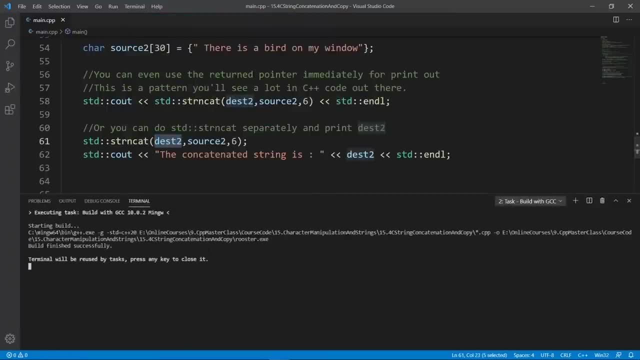 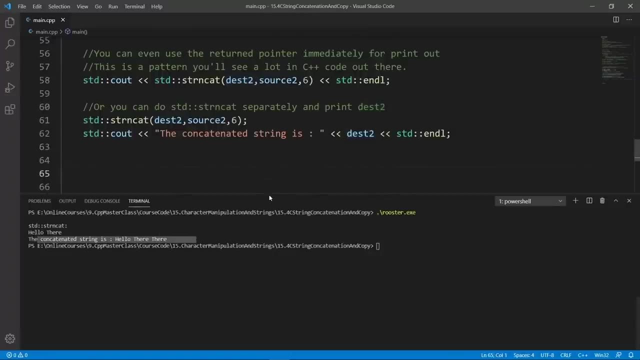 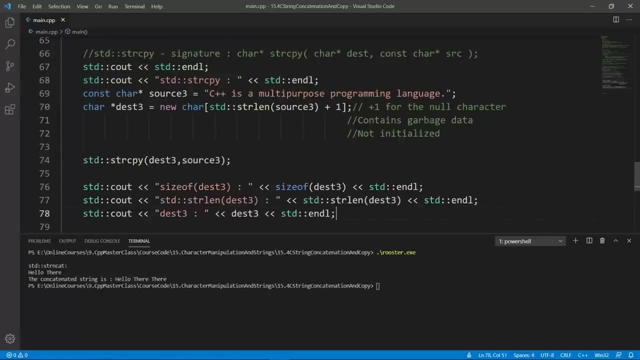 build this to build with gcc. the build is going to be good. we're going to clear and run roaster and you're going to see that we have hello there twice here and this is exactly what we expect. we are going to comment this out and we are going to go down and look at str cpi. i should say str cpy, which is: 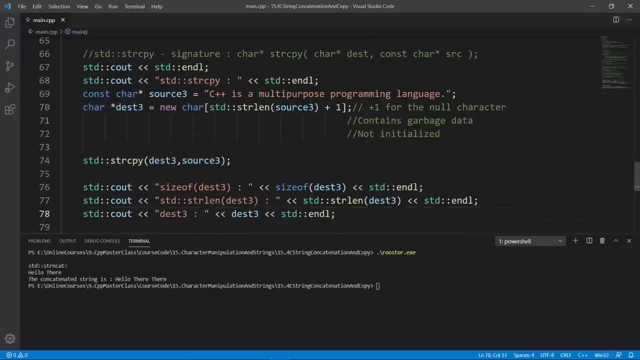 going to copy stuff from the source and paste those in the destination, and one thing you should know is that the copy is going to happen starting from the start of the destination array. here we have two arrays. one is called source three, the other is called destination three. destination- 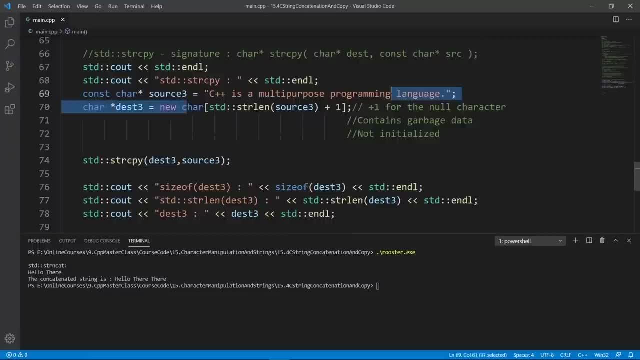 three is set up on the heap using the new operator. so it is a dynamic array and you see that we make sure that it is the same size as the source. we are using strlan to figure out how many characters we have in here, and remember that strlan doesn't account for the null character. 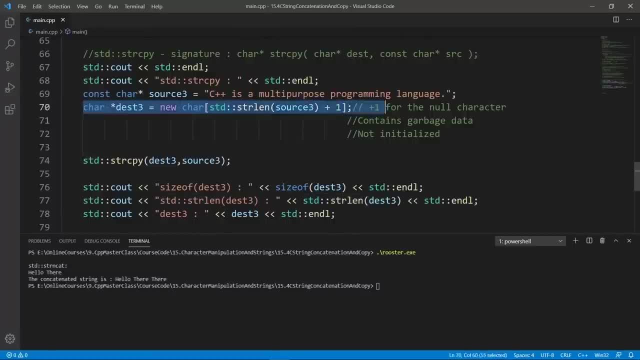 so we are adding one to account for the null character. that's what we are doing here, and after that we are going to do std, str, cpy, and what that is going to do is copy stuff from source to destination character by character. so we are basically going to have this guy pasted into. 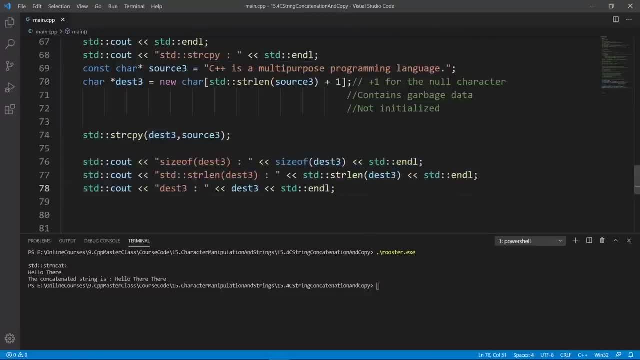 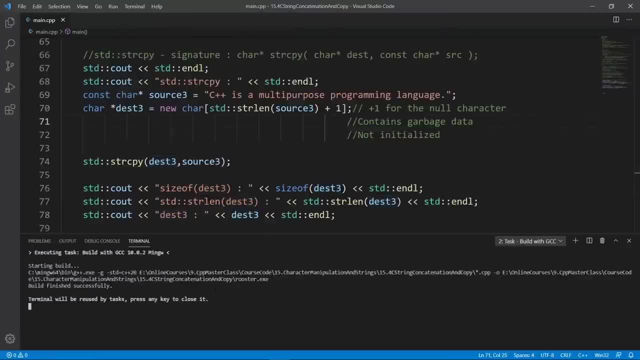 destination here and if we print things out, we're going to see that destination contains the same thing as source here. if we built this with gcc, let's do that. the world is going to be good. we can clear and run, rooster and you're going to see that the destination has exactly. 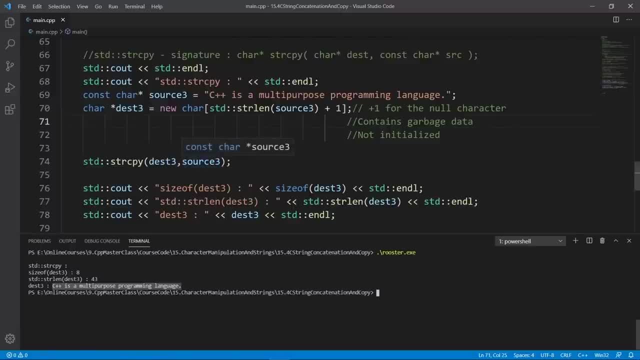 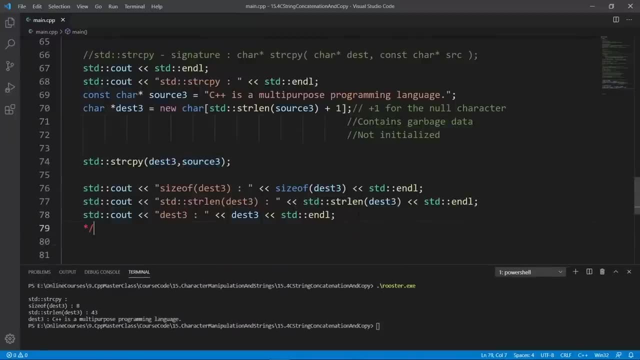 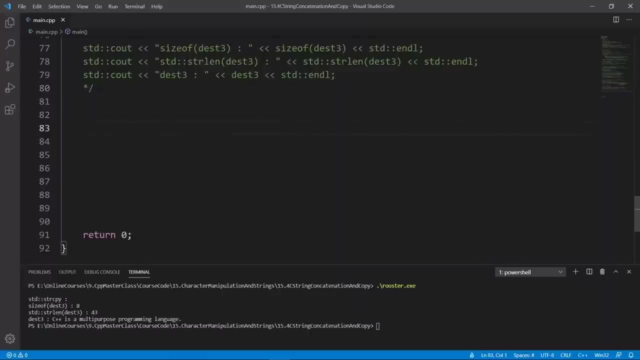 the same thing we had in the source, and if you need to copy stuff from arrays, hdr, cpy is going to be very helpful. we are going to comment this out because we still have a few things we want to see, so let's comment this out. we are going to go down and see that we can also use. 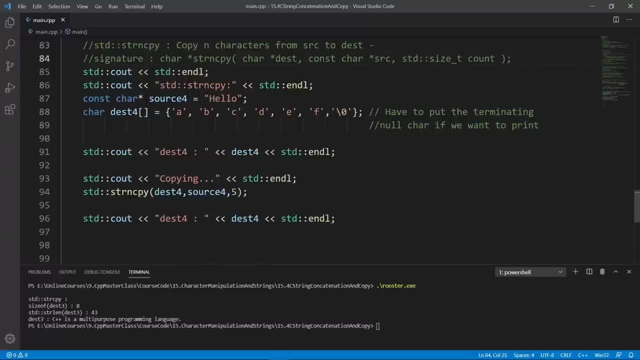 a another version that allows us to specify how many characters we want copied from the source. okay, in this example here we are using std, str, n, cpy, and this n here means that we can specify the count of characters. we do whatever the current function is doing here. okay, so we. 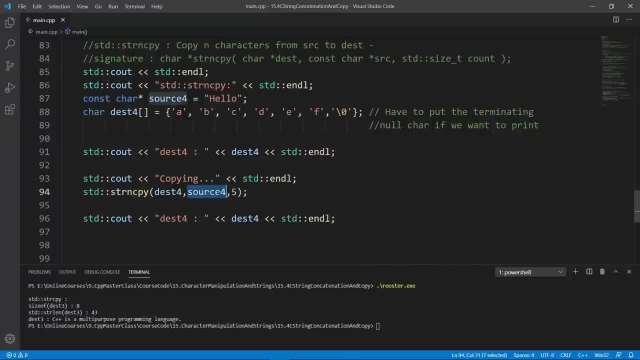 are specifying. i want five characters copied from source and i want those pasted into destination here. that's what we are saying here, and the source is going to contain hello. destination is going to contain the world and the copy is going to happen starting at the first index here. so we're going to 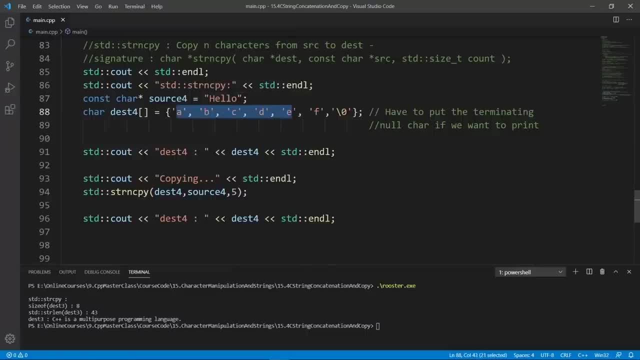 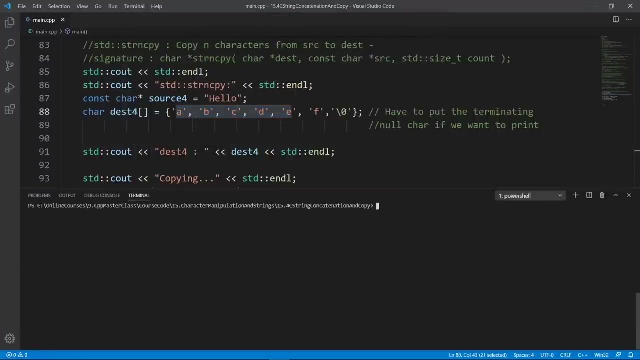 have hello, override whatever we have in a, b, c, d, e, because that's five characters here and dest is going to contain hello f. if we print it out, let's build this and see if that's what we're going to get. we're going to build with gcc. the build is going to go through. we are going to clear and 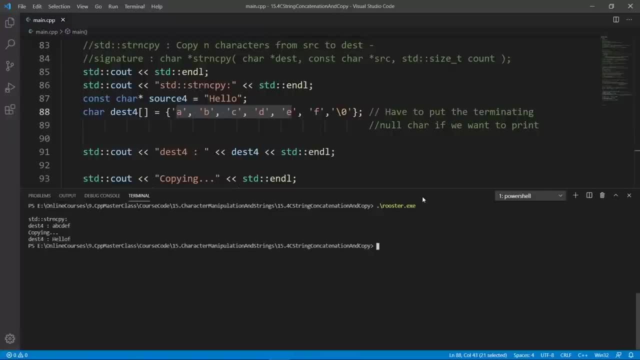 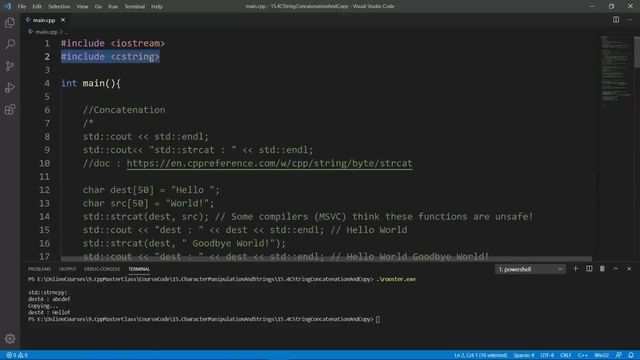 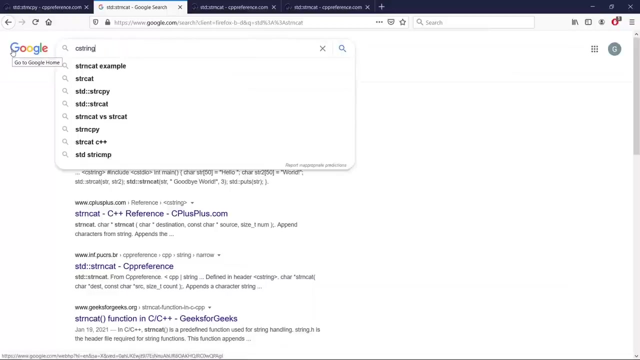 run rooster and you see that that's exactly what we have here. okay, this is how this methods work. there are many more functions you can use from the c string library and again, if you want to see a list of them all, you can go through your favorite search engine and search for c string. 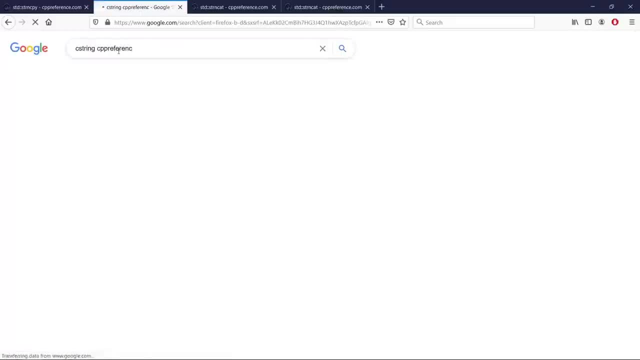 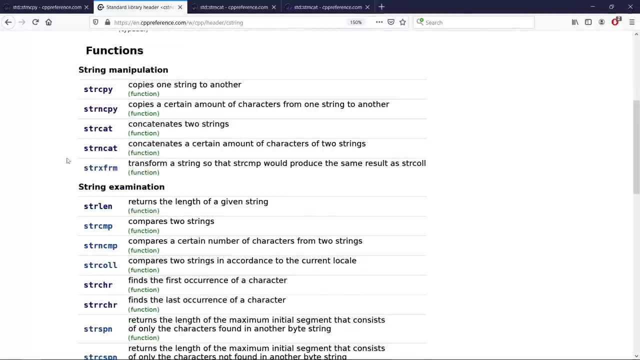 and we can specify cpp reference here. let's try and do that. okay, we can find a link to that. we can click on that and it's going to open up and show us many more functions we can use. and if you need to know about a special function, you can click. 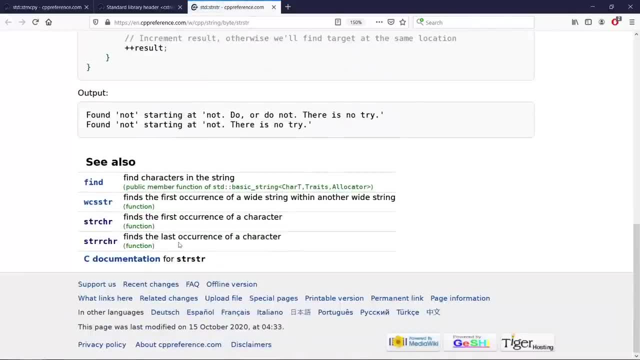 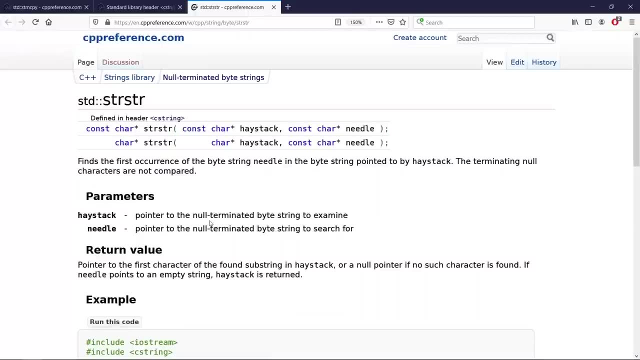 on it and see what it does, and if you go down, you're going to find even an example of how you can use it. for now, we are going to stop here in this lecture, and this is actually going to be the last lecture we see on c strings. in the next one we're going to start and look at std string, which 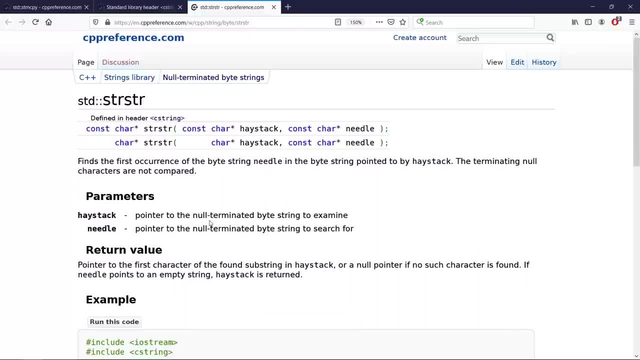 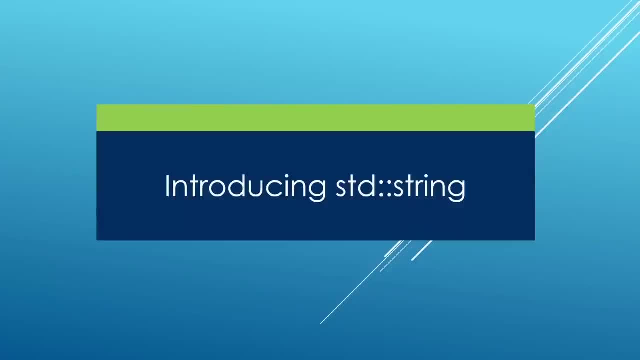 is a compound type that makes working with strings very easy in c plus plus. go ahead and finish up here and meet me there. in this lecture we're going to start and learn about std strand, which is a type of string that's going to make it super easy to work with string data. we have seen many ways we 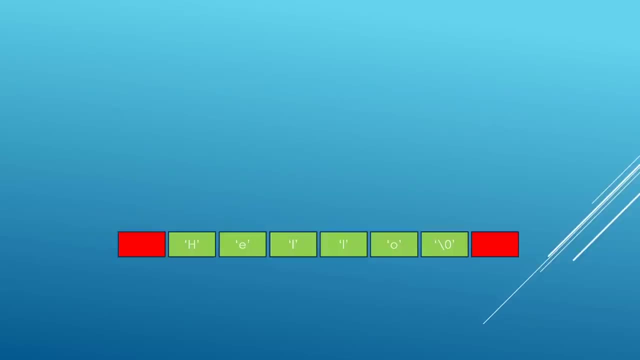 can work with character arrays by now. we can use row arrays, we can point to them with pointers, we can even allocate arrays on the heap. but all these character arrays had a few problems that are really a pain in the neck to deal with on a daily basis. one of those problems was that: 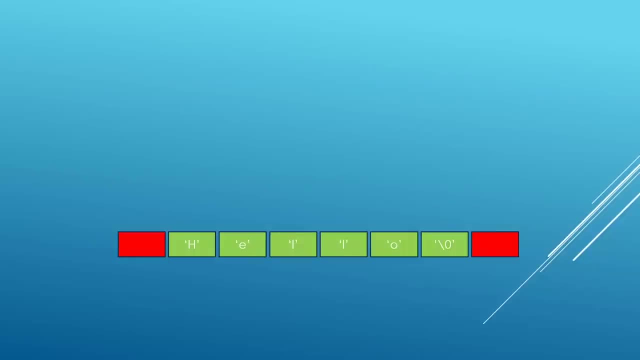 you had to keep the sizing check. you have to know how many elements you have in the character array and that was defining the bounds that you can work in. if you go over bounds, we have seen that that can cause crashes of your program and you don't want that. another problem was that we had 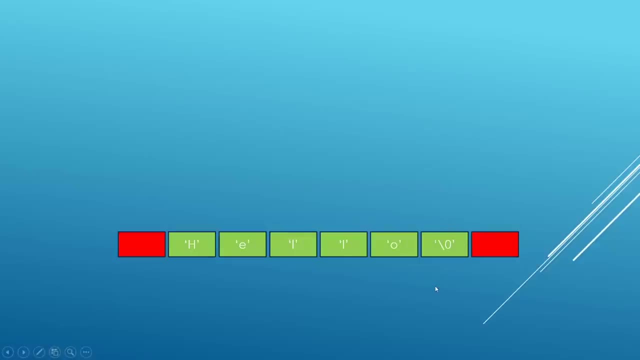 3d to remember to keep track of the null character. if we don't have it in place, we're going to have problems when our string is printed out, and it's really annoying to always have to think about these little details when all you really want is to store a string. so c plus, plus. 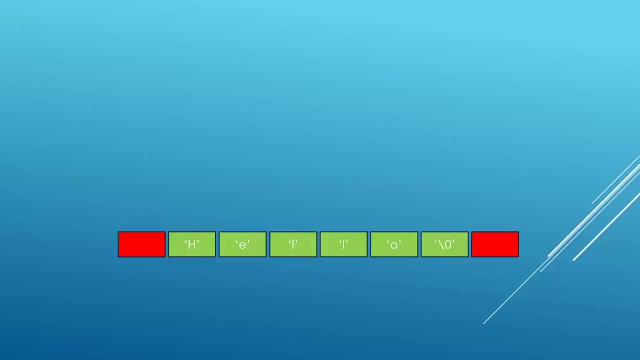 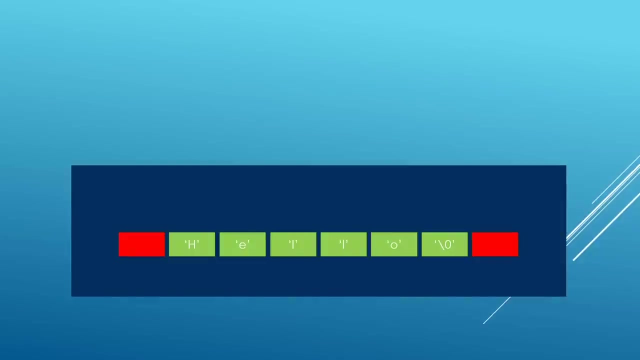 offers a high level type that we can use and it is going to hide all these little details and a ground and all we have to do is put in our string and use it, and we can be on our merry way and do whatever we want to do with string data in our c++ application. so that's what we're going to. 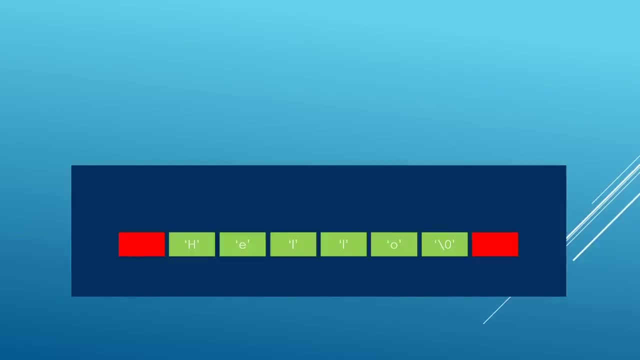 do? we're going to have a type that is going to wrap on top of the ugly array computations we have been doing on character arrays. we're going to call that std string and we're going to be able to many of the things we were doing with c strings, but in a much better way. we can concatenate. we. 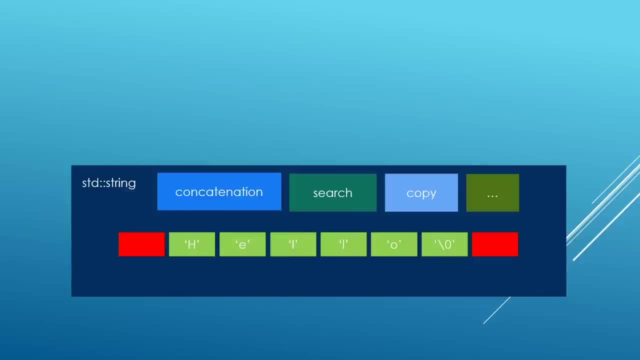 can search, we can copy, we can do all kinds of crazy things really. but it's going to be in a way that you don't have to worry about these little details about array bounds, the null character. you're going to just use it for what you want, which is storing character or text data. okay, 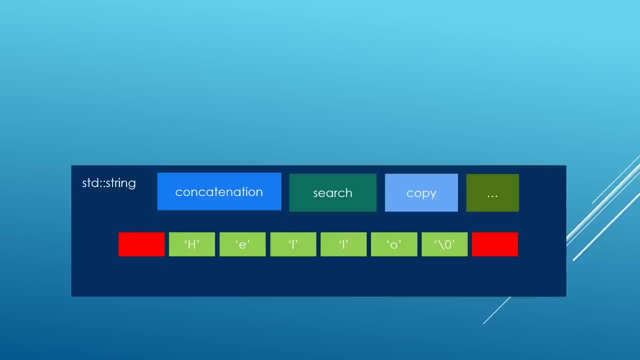 so that's what we're going to be doing in the next few lectures. we're going to be learning about std string and how you can use it in your c plus plus applications, and it's going to make your life a whole lot easier. we are going to stop here in this lecture. in the next one we're going to see how you 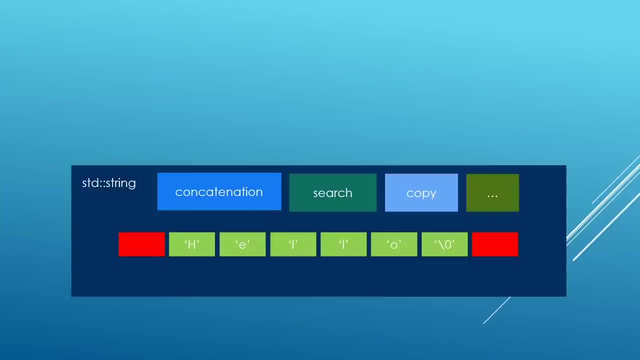 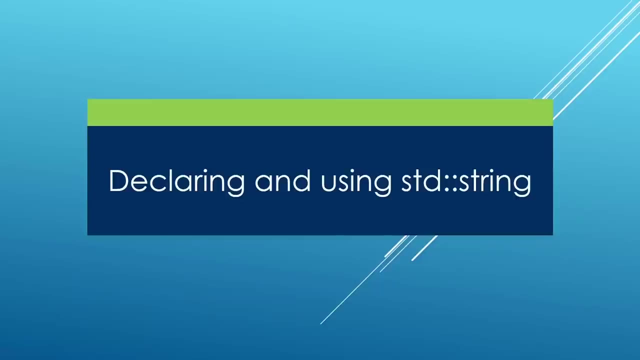 can declare, initialize and use std string in your c plus plus application. go ahead and finish up here and meet me there. and this lecture we're going to see how you can declare and use std strength in your c plus plus applications. std strength is a type that is going to wrap on top. 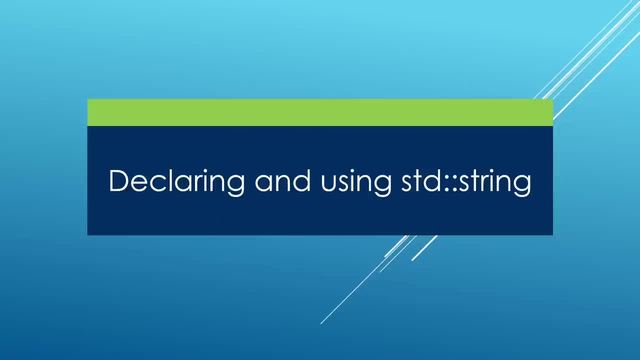 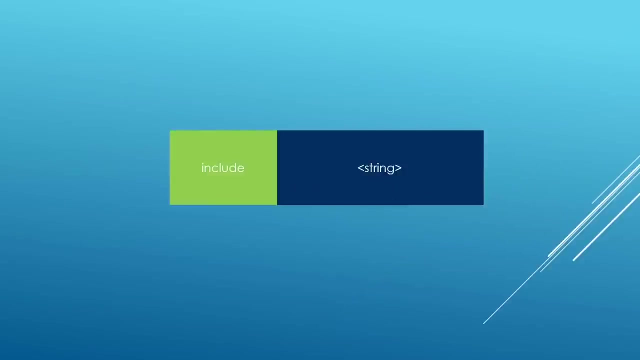 of arrays and give us a really nice interface that we can use to store string data without having to deal with the ugly little details like keeping track of array bounds, remembering to keep in check the null character and things like that. to use std strength, you will need to include the string library and after you do this, you 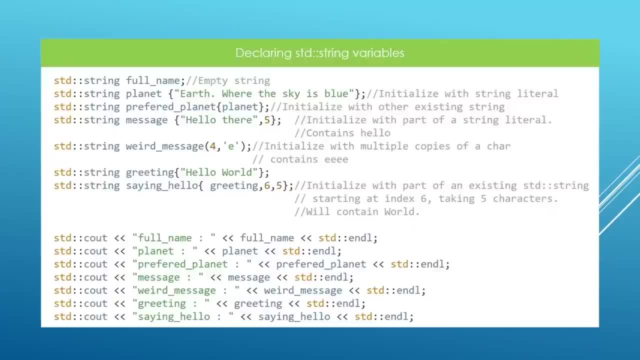 can declare and use your strengths just like this. here we have a series of examples just to get you started on this. you declare your strengths just like you declare any other time. you specify the type on the left. the type is going to be std string. by the way, you'll have to remember to use std colon colon. 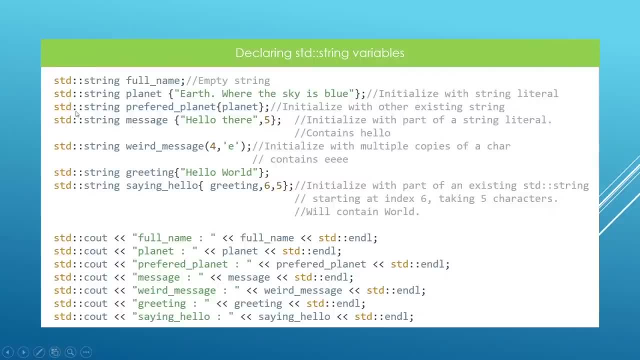 like this, and we will have a chance to explain why in a few chapters ahead. but for now we're just going to think of std string as our type. so we declare a string type, we call it full name and we can leave it like this uninitialized, and it is going to be an empty string. we can also put: 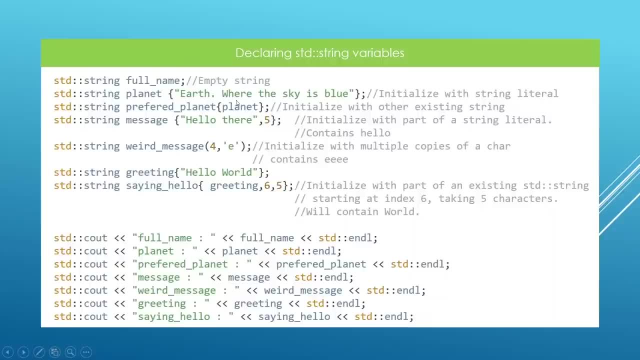 in our string and initialize that with a string literal, and it is going to work. another way of doing this is initializing a string with another string, which we are doing down here. we can also set up another string and initialize it with part of another string literal. so, for example, message: 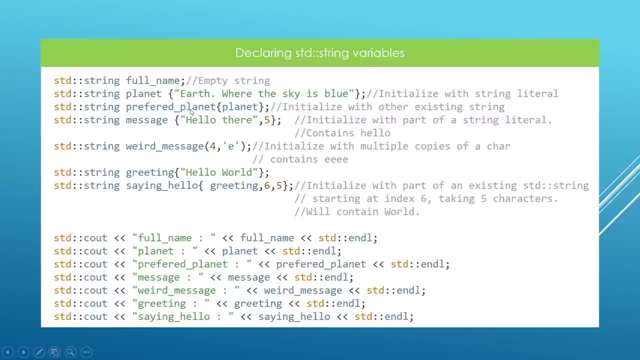 here is going to be hello and it's only going to grab five characters from this string literal. this is something you might want to do, if it makes sense, for whatever application you are doing here. we can also initialize our string with multiple copies of one character and this is the syntax. 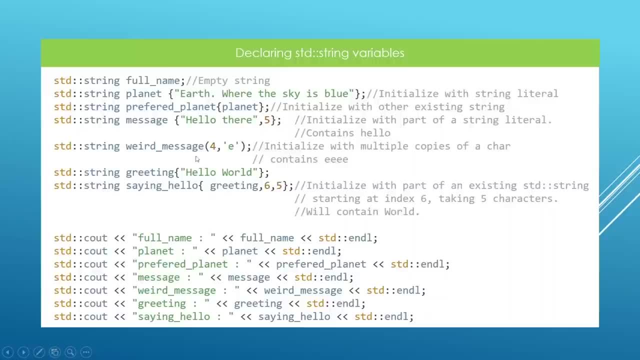 to do it. you say the name of your variable, you say however many times you want the character repeated and you say which character it is. just like this, we can also initialize a string with part of another existing string. so, for example, here we have saying hello and it is initialized with part. 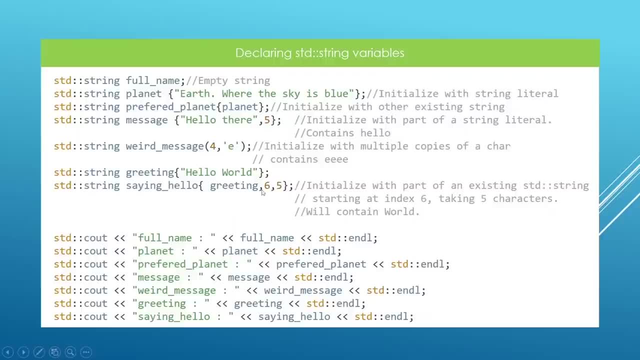 of what we have in greeting here. so we're going to start at index six, which is going to be zero: one, two, three, four, five, six on the w here and we're going to grab five characters. so one, two, three, four, five, and that's what we're going to use to initialize this saying hello here. 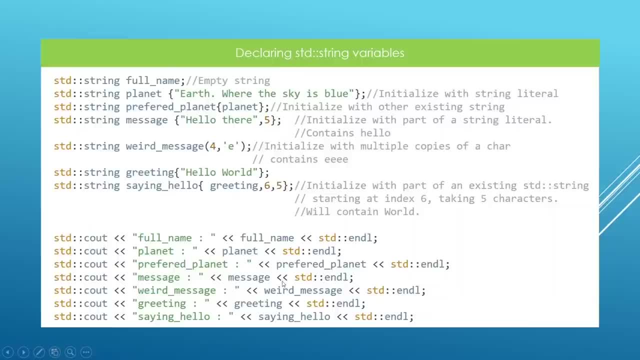 and if we print it out, we're going to see that this is going to be exactly the case. so hopefully you can see that it is easier. you don't have to use pointers, you don't have to use arrays and the best part is std string can grow automatically, if you happen. 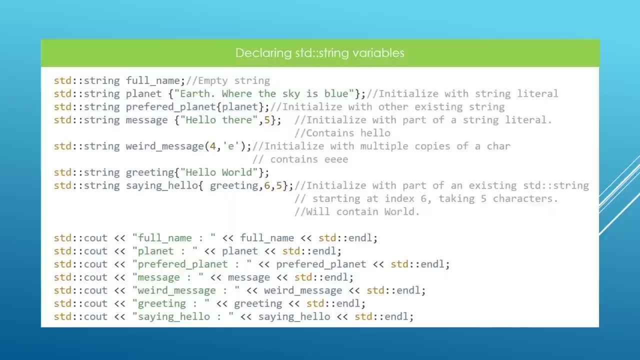 to store in more characters than you initialized it with in the first place, and that's pretty cool. so now we're going to head over to visual studio code and play with us. that you can see for yourself. okay, here we are in our working folder. the current project is declaring: 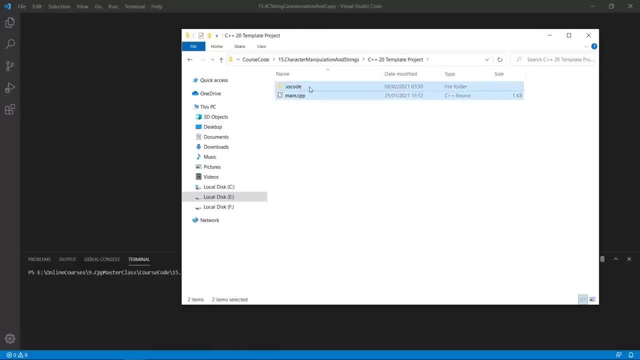 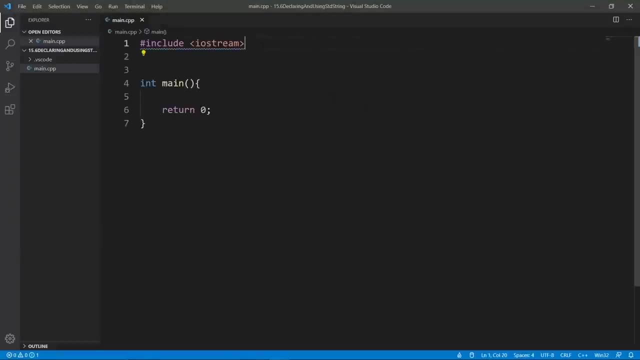 and using std string, which is what we are doing here. we're going to grab our template files pretty quick and we're going to go and install in the files and we're going to open the folder and we're going to include the string library. let's do that, okay, this is how we do it, and now that we have it, 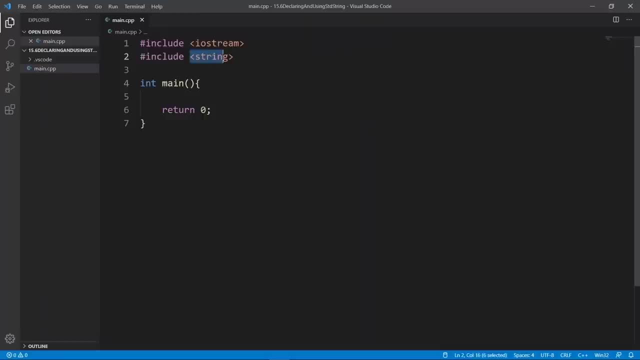 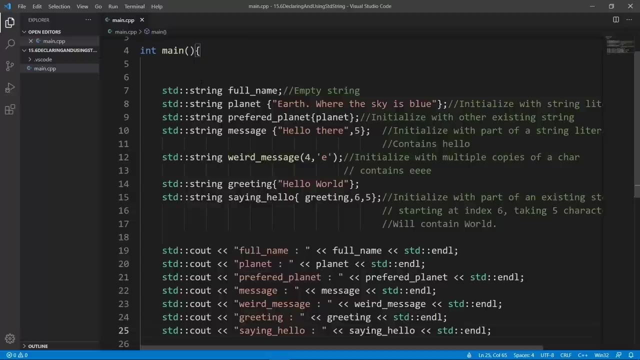 included in our project. we can start declaring and using std string types in our c++ program. we are going to go down and put in the code to play with this a little bit so you can declare an empty string like this and it's not going to have anything inside. you can declare a string and. 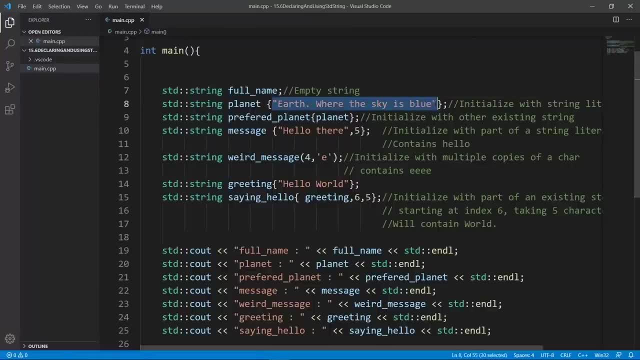 put in a string, literal, like we are doing here, and std string knows how to handle this, so it's going to store it inside using a character array, but we don't have to really worry about that character array because we don't have to worry about that character array, because we don't have 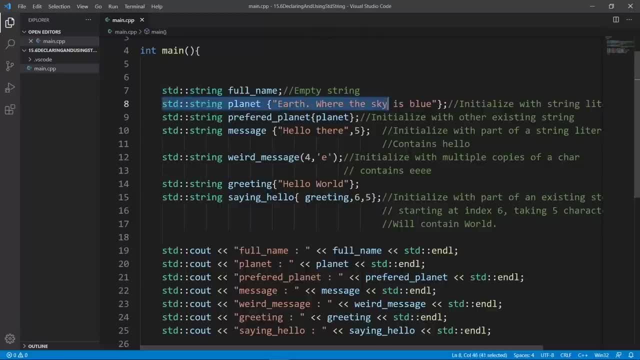 is going to work. we're just going to use std string here. we can set up a string using another string in our initializer. like this, we can also use part of a literal to initialize the string. so, for example, this string literal, here we're going to grab part of it and we're going to grab. 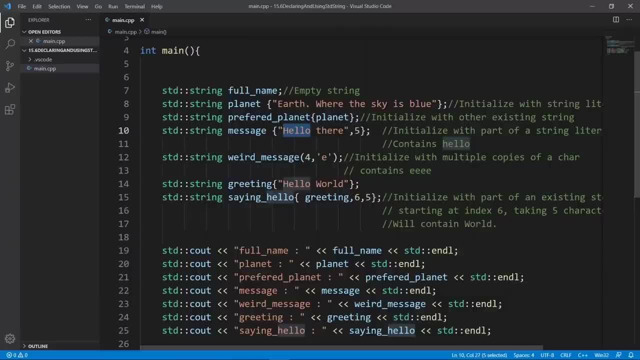 five characters and use those to initialize our message std string here, and this is pretty cool. we can also use multiple characters to initialize a string like this. we say however many copies we want of this character in this string here and it is going to be exactly what we want. so it's going to be four e's in this weird message string and we can. 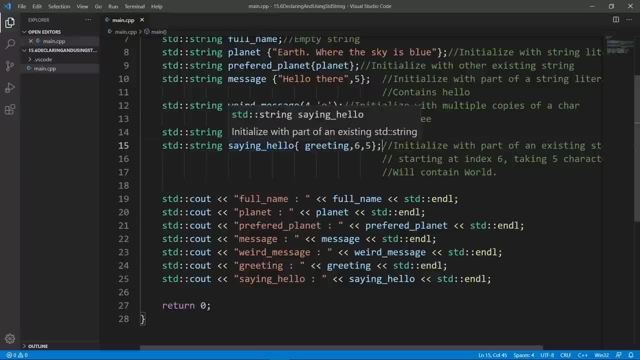 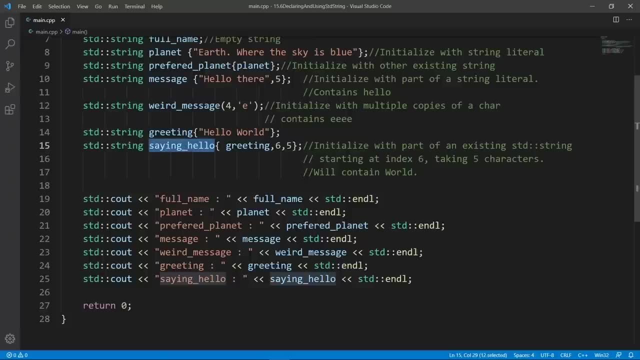 initialize a string with part of another string and this is really cool and it may come in handy in many applications. so, for example, here saying hello is going to contain world here, and we are saying that this is what we want by saying we want to start at index six in this string. 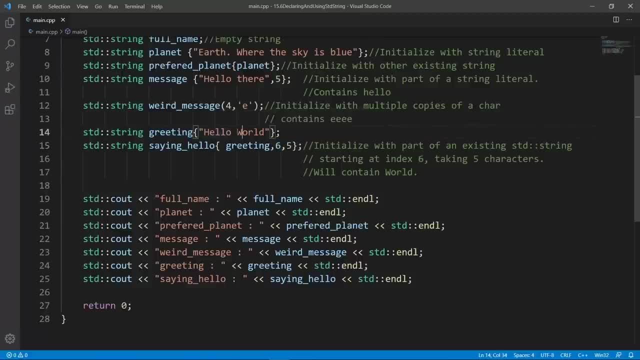 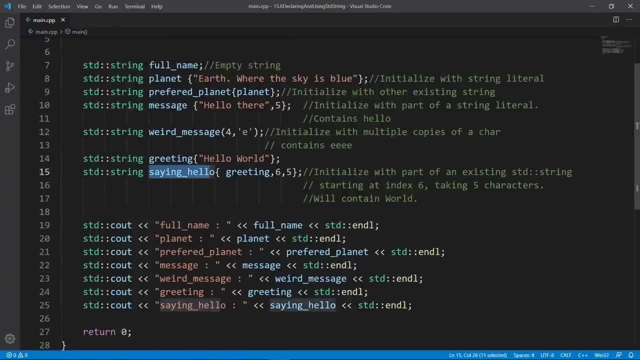 here. so if we go zero, one, two, three, four, five, six, this is going to be our character at index six and from this index we're going to grab five characters. so we're going to count one, two, three, four, five and that's going to be what's stored in this string here. and if you don't believe me, 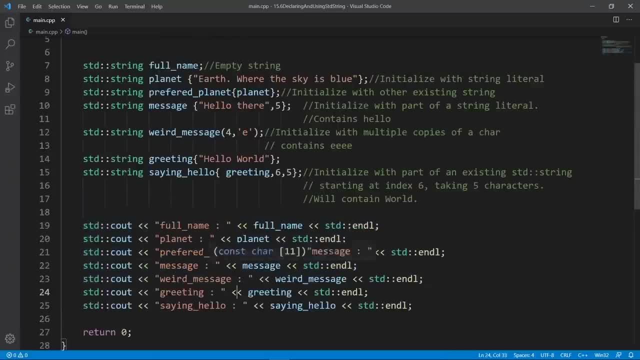 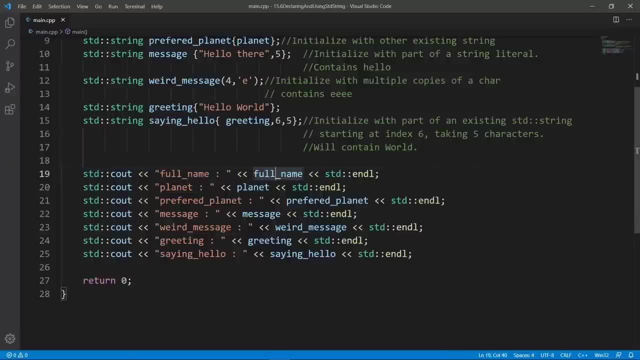 we can print all these things out and they are going to be exactly what we expect, and by this you can even see that we can print std strings using stdc out very conveniently like this, and this is very cool. okay, so we can try and build this with gcc. the builder is going to go. 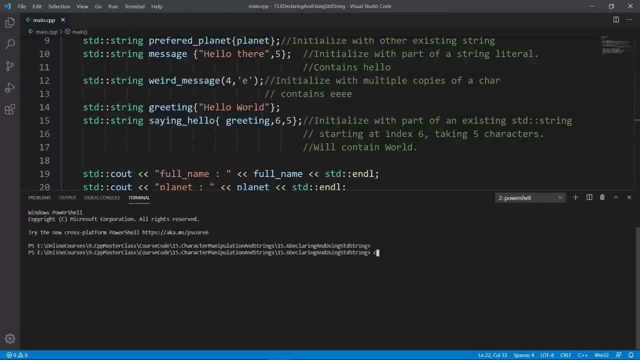 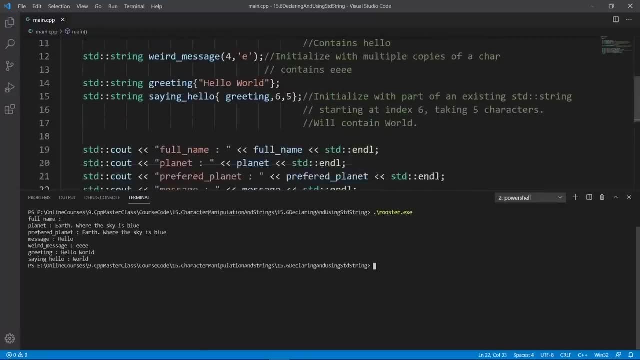 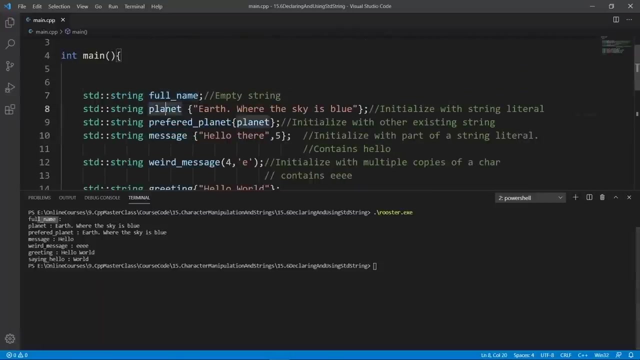 through. so we're going to bring up a terminal so that we can run this and we're going to clear and let's see what we see when we run rooster here. so we're going to print the full name. the full name is empty. okay, so we're not going to see anything because it is empty. we're going to see planet. 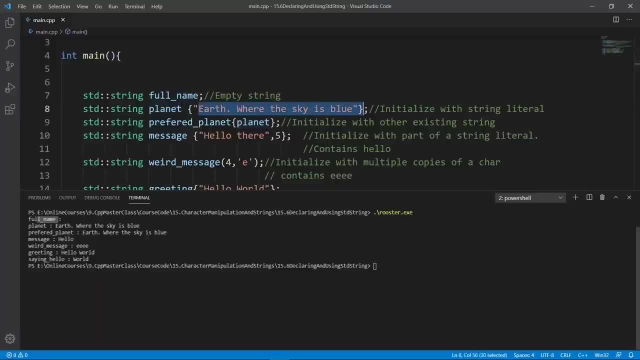 planet is this thing we have in here, planet where the sky is blue. so this is what we expect. we can, uh say preferred planet and put in the text for the planet here. so we're going to get the same thing here. and if we have a message and say hello there and grab the first characters in 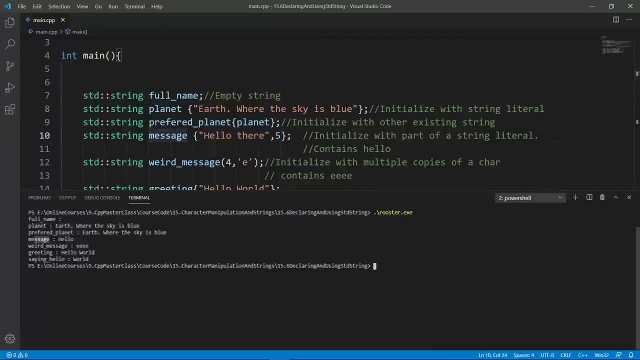 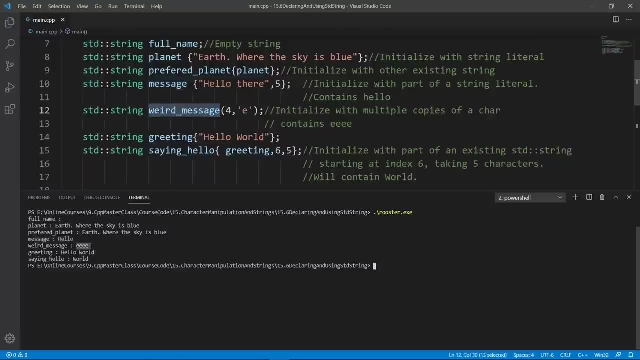 this string literal message is going to say hello, which is what we are saying here. let's go down and look at weird message. it's going to be for ease, which is what we have here, and we can initialize saying hello with part of what we have in greeting and we have targeted this. 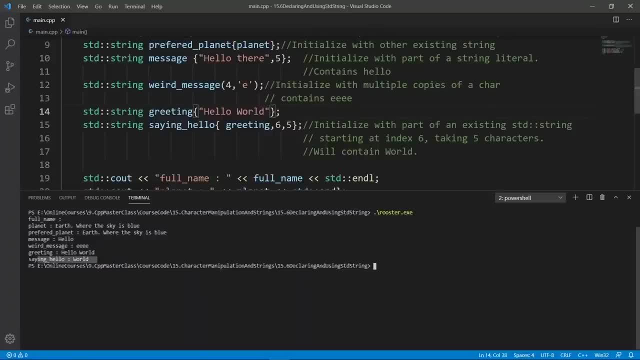 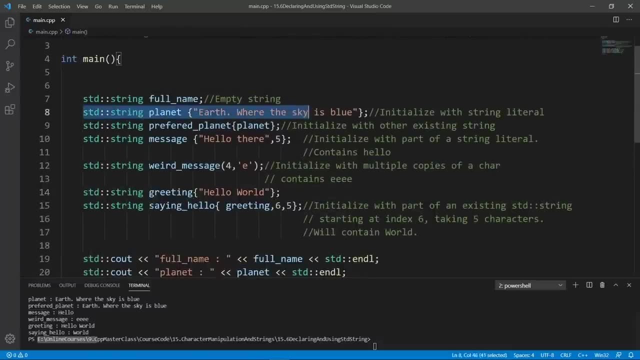 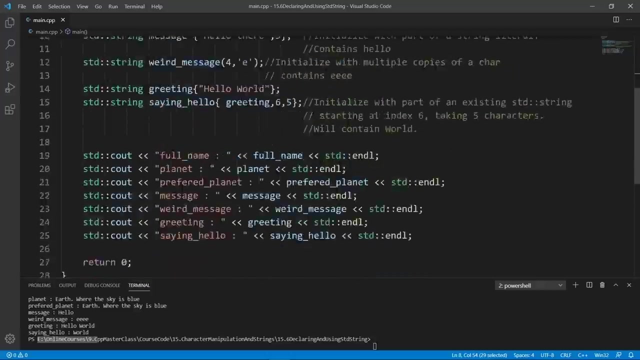 word string here, and it is what we see here, and this is pretty cool. the good thing about std string, however, is that you can store in more characters than we initialize this guy with. so, for example, here we have this message here, but we can say: planet, let's go down here and say it, we're going. 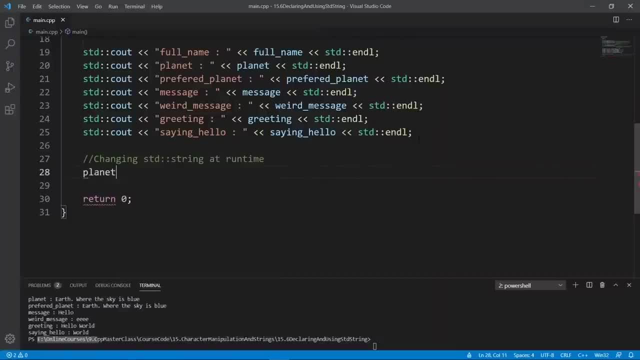 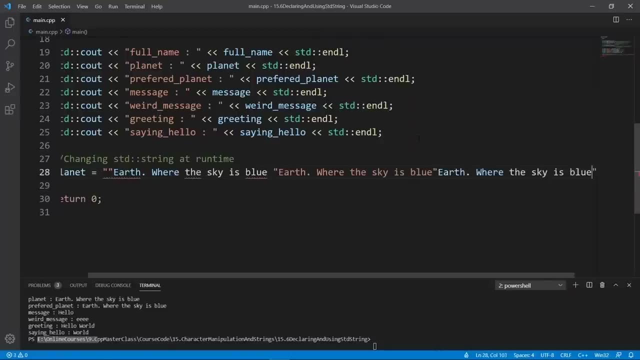 to change std string at runtime. so we're going to say planet and we're going to assign something to it, we're going to put in whatever was in there first and we're going to paste that in multiple times. let's do three times. i think that's going to be enough, or we can even bring this back. 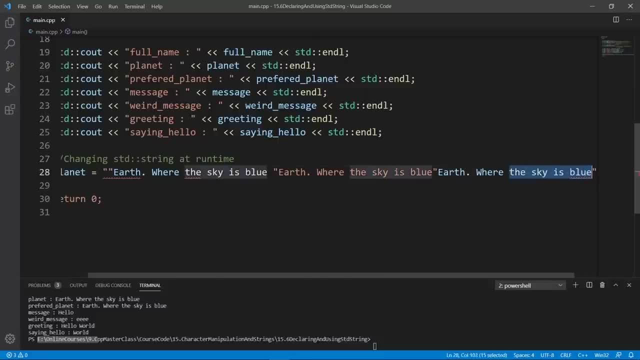 so that we see the entire thing here doesn't really matter. all we want is for this thing to be larger than it was initially declared in uh planet here. so we're going to remove these quotes because they are making things ugly for us, and now it's going to be a valid string. let's wait. 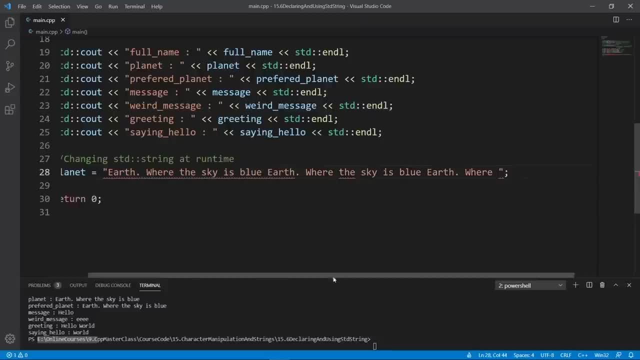 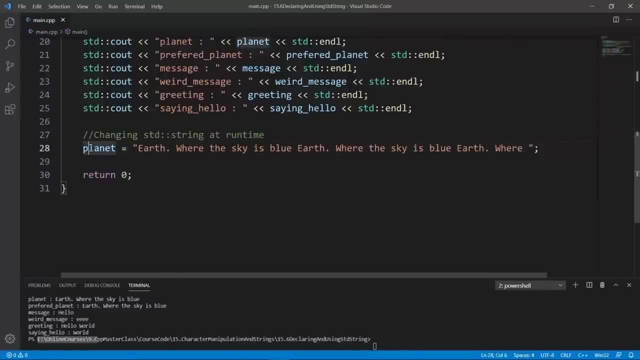 for visual studio code to realize that and it's going to remove these squiggly lines. we are good. std string is automatically going to take care of the logic to make this string grow. we don't have to worry about that. and if we print planet now, we're going to see the same. 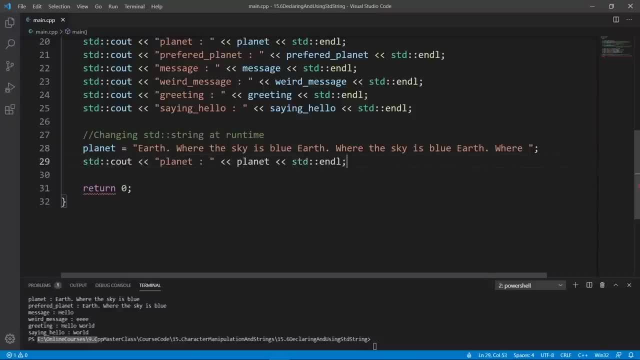 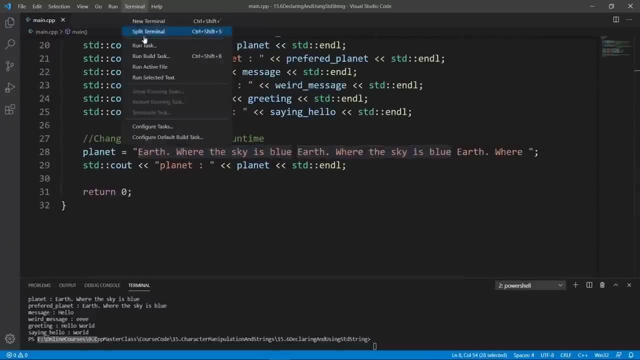 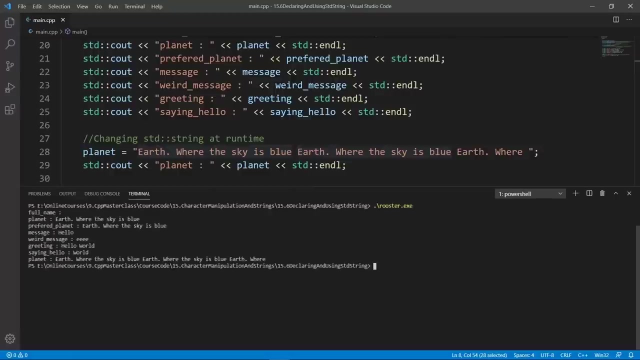 details and taken care of. okay, this is really cool and it makes it super easy to work with text and string data, like you see here. so let's build again so that our changes are reflected in our output. we're going to clear and run rooster and we're going to 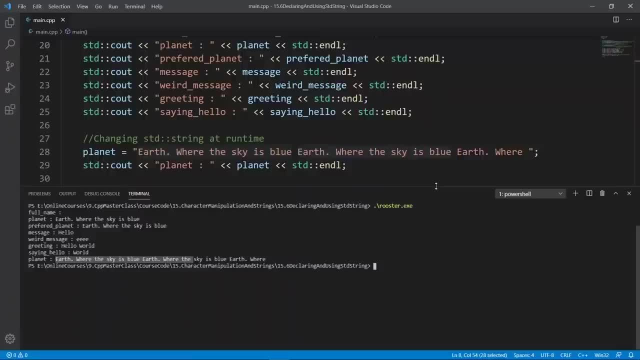 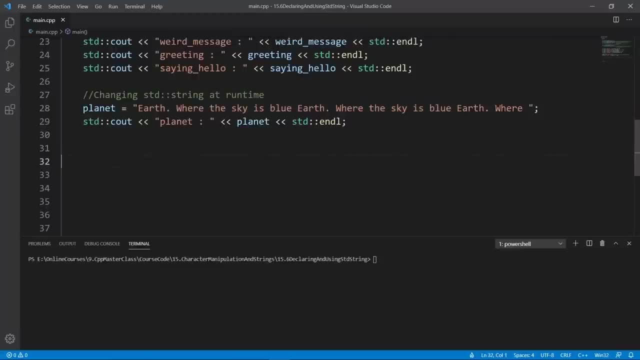 see that planet is now really large. okay, we can change this thing, the size of this thing, at run time, and this is something we couldn't do with arrays. so, for example, if we go down here and use a row array to do something like this, this code is going to run. but try to think about what. 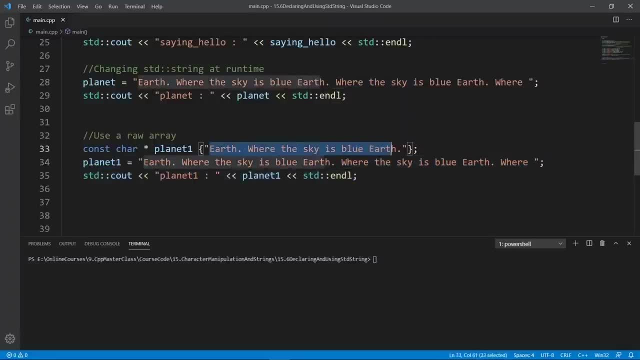 is really happening here. we have an array which contains this text here and it is pointed to by this const car pointer that we have, if we try and do an assignment like this. this is really going to be to make it point to another character array in memory, and this piece of memory here is basically: 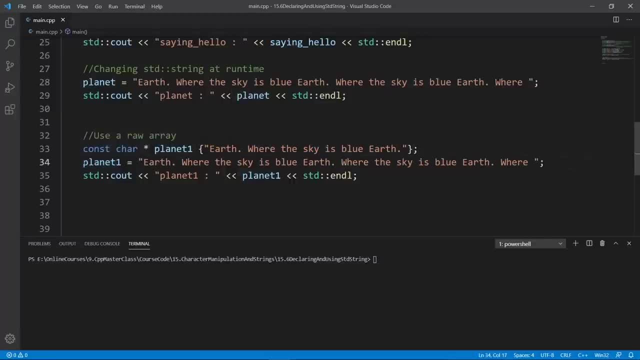 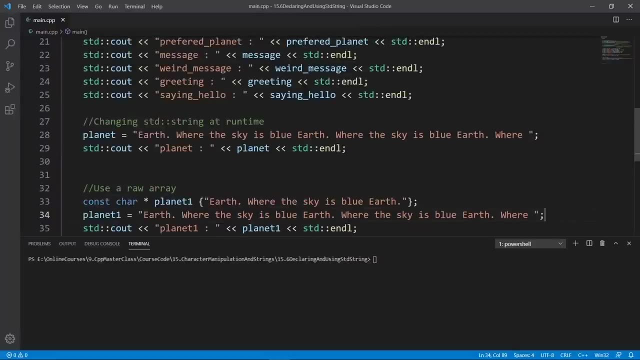 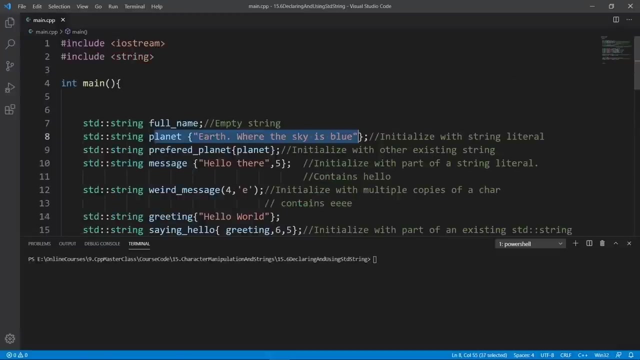 going to be wasted because we think we have our planet string in here. this is not the case with std strength, because std strength, when we do something like this, the initial memory that was allocated to store planet here is going to be returned to the operand system and a new memory. 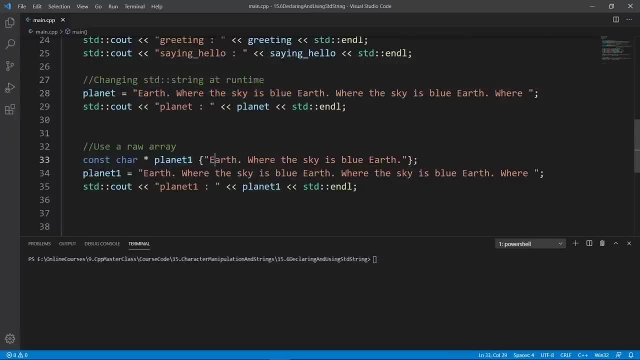 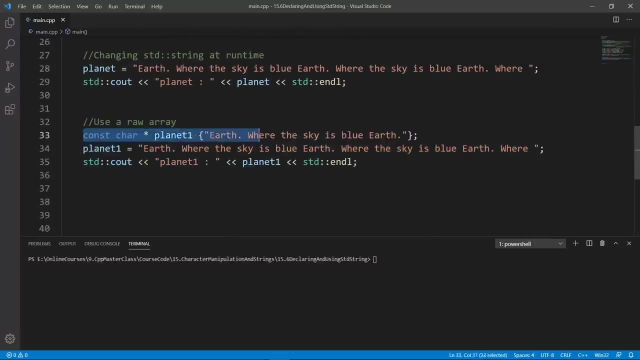 is contained, this new thing. so the waste we're doing here by just leaving this in memory and not using it is not being done here. so if we try to print we're going to get the same output. but inside, in how our memory is managed, std string is better in that the memory that was used to 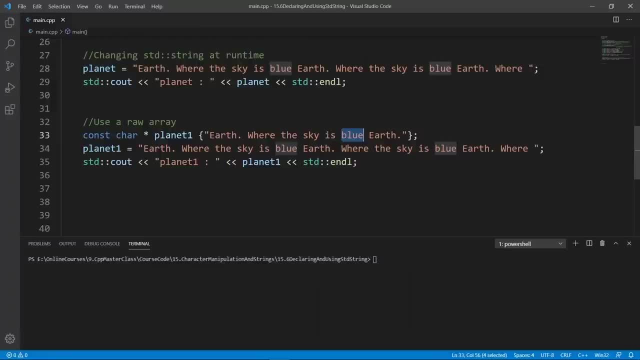 initialize. this guy is not wasted out here with array. what we really are doing is just make this planet pointer point to another string, and leaving this to be wasted in memory is what we are doing here, and we can avoid that with std strength in this lecture we're going. 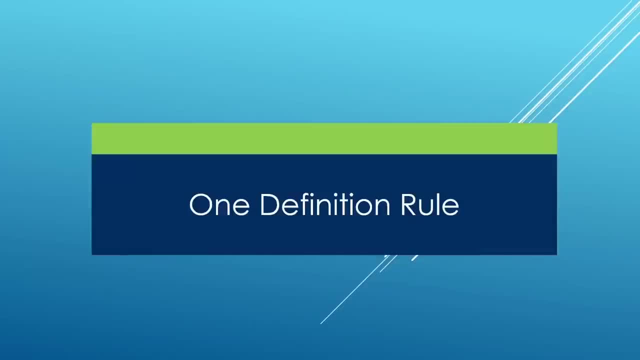 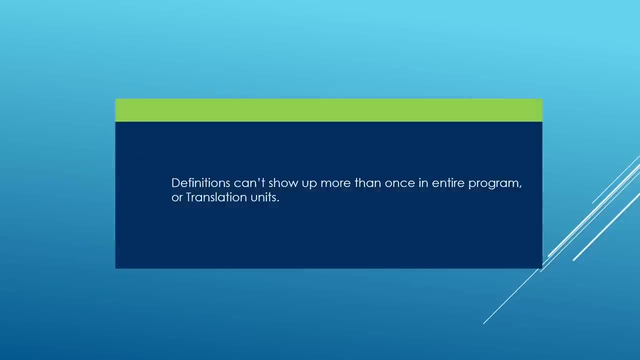 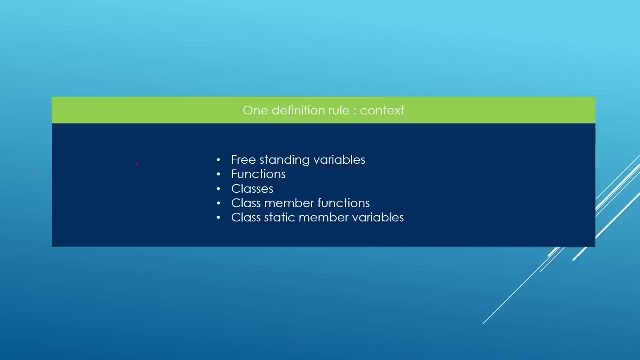 to learn about the one definition rule, and this is a rule that says definitions can't show up more than once in your entire c plus plus program, or in some cases, a definition can show up more than once in a translation unit. we are going to look at the one definition rule in the context of 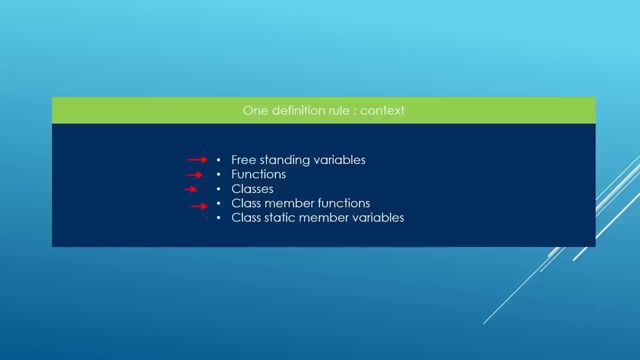 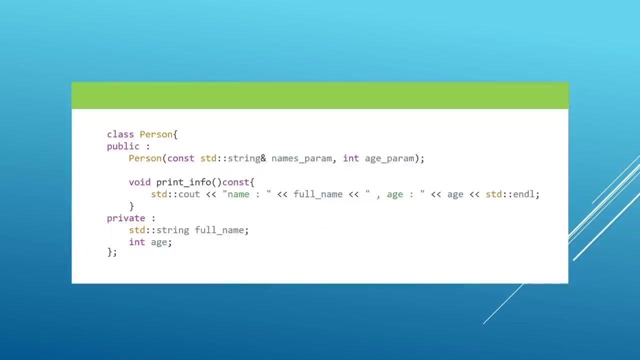 freestanding variables, functions, classes, member functions and static members in our classes. in most cases a definition can't really show up more than once in your entire c plus plus program. but we have exceptions to this rule and the exception is for classes. a definition for a class can show up in multiple translation units and the reason is: 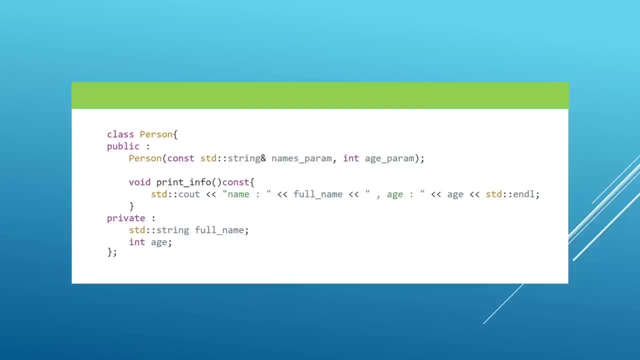 we need to create objects of those classes, so each translation unit really needs to see the definition for the class and- And we are going to try and make this super clear with examples- once we hit Visual Studio Code. Okay, so it is time to head over to Visual Studio Code and shed some more light. 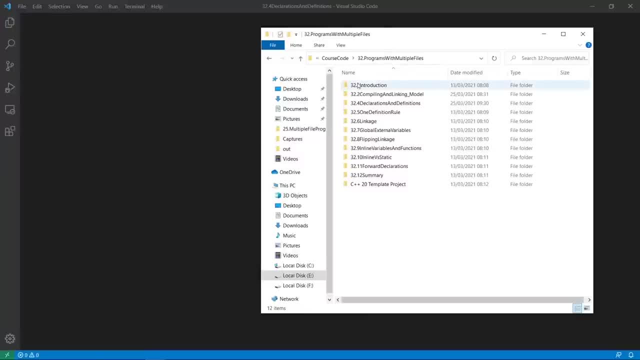 on the one definition rule. Here we are in our working folder. The current project is one definition rule. We're going to grab our template files, like we always do, We're going to put them in place and we're going to open this little guy in Visual Studio Code. Let's do that, We're going. 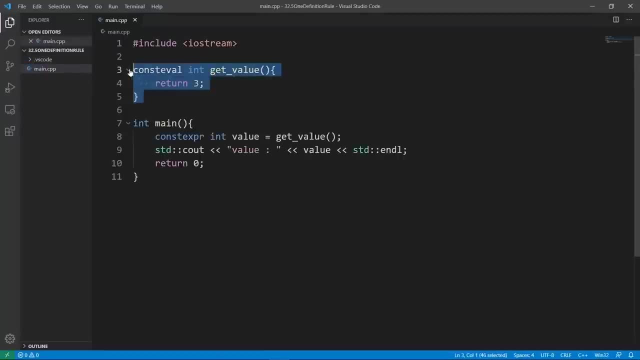 to drag and drop and we're going to have our main CPP file here. We're going to clean it up. That's what we always do. And now we want to explore the one definition rule in the context of variables. So we have a freestanding variable here And that's going to be the same variable. we 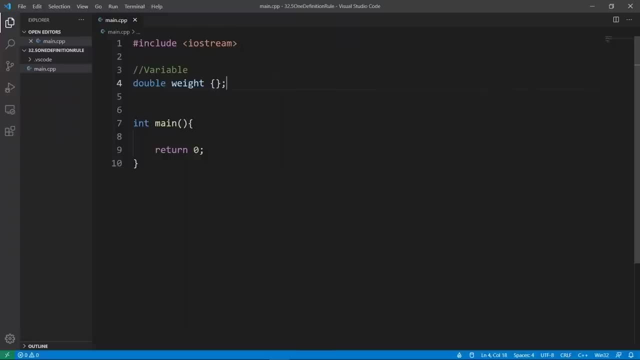 had in the last lecture. We're going to initialize this And this is really good. We can use it. We can go in main and use it however we want. We can print the way And if we want to run this program, it is going to work. But the one definition rule says we can't have more than 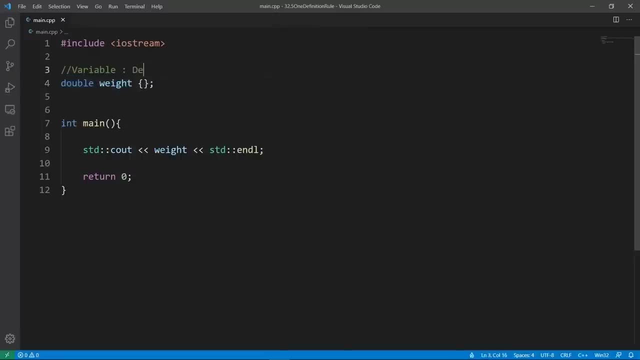 one definition for anything And for this variable. here we have seen that this is both a declaration and a definition. So we can't have more than one definition for the weight name here, For example, if we try and grab it and copy and paste it here. So we're going to try and build this program. 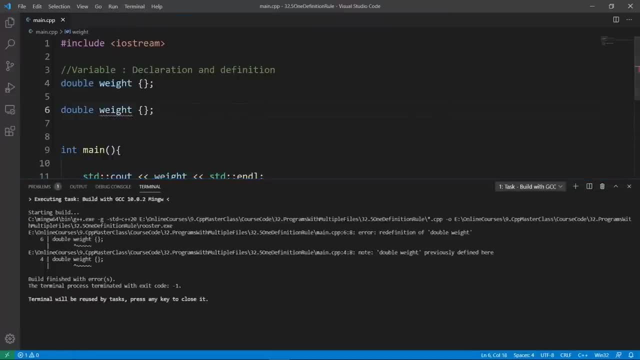 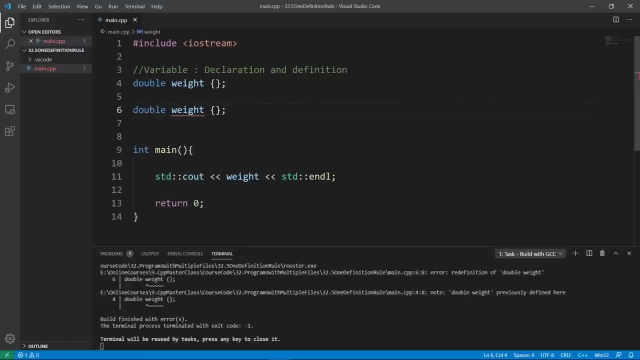 We're going to use GCC, We're going to see that we have a problem And the problem is going to say redefinition of double weight, And it is not going to help even if you take this and put that in another file. So let's create another file to really show you that we're 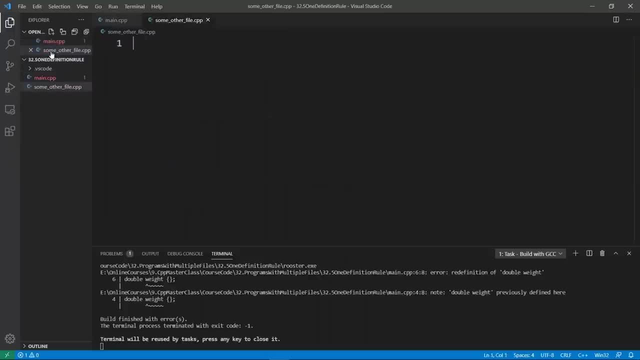 going to call it some other file, that CPP, And we're going to grab our redefinition and move that there. And you're going to see that if we try and build this program we're going to get the same problem. We're going to have redefinition, So we're going to see. 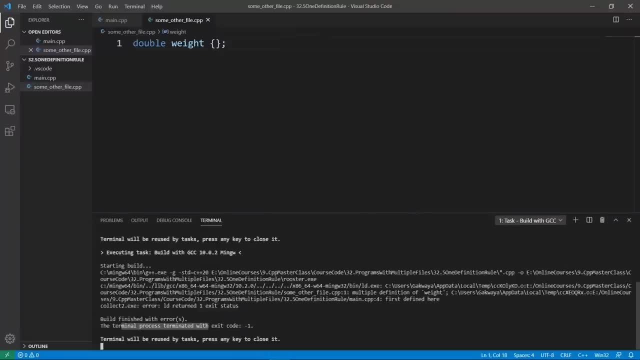 what is the problem here? The compiler error is a little bit different, but it is going to say multiple definitions of weight And it's going to say one is defined in the main CPP file. So this is a linker error. This was code by the linker because the redefinition is showing up in multiple. 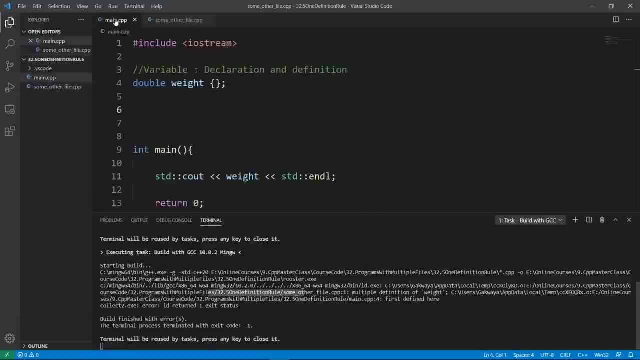 files. So the linker was linking this program and it needed to see a definition for weight. And it has seen one definition in the main CPP file And it has seen another definition and some other file And this is a problem. The linker doesn't know which one to choose. 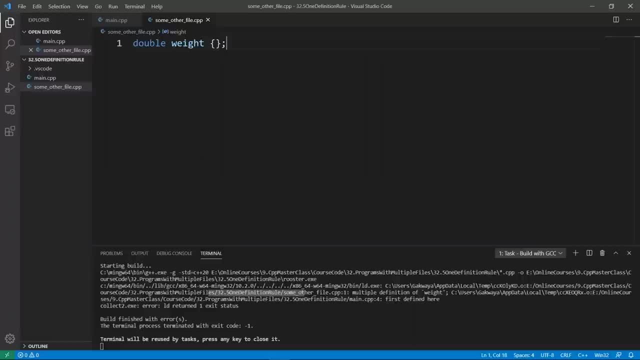 So it's going to throw an error And you can't really have multiple definitions for a variable in your C++ program. And this is the one definition rule in the context of freestanding variables like the weight here. But this is the same in the context of functions. If we go down. 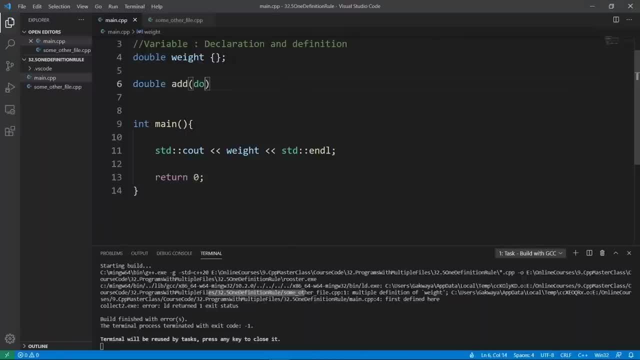 and put up our add function here. we're going to say double A and double B here And we're going to put the definition below the main CPP file. Let's grab this. We can copy this and put this in the code here. We're going to remove this little thing. We don't want it. We're going to put in our body. 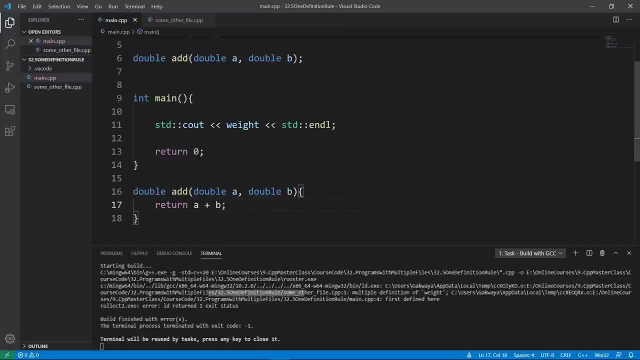 And we're going to return A plus B here. Okay, so this is our function. It is working. We can take out what we had here because it has served its purpose. We can say double result And we're going to add up 10 and 20, like we did in the last lecture. No problem, And we can try and 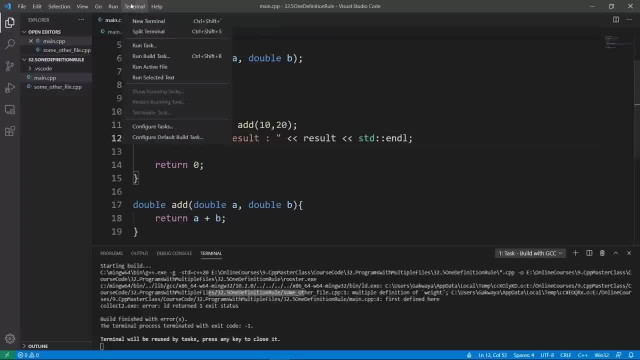 print this out And we're going to put in our body And we're going to put in our function And we're going to print out our results here. If we build and run this program, it is going to work without a problem, because we only have one definition for the add function. What is the problem here? 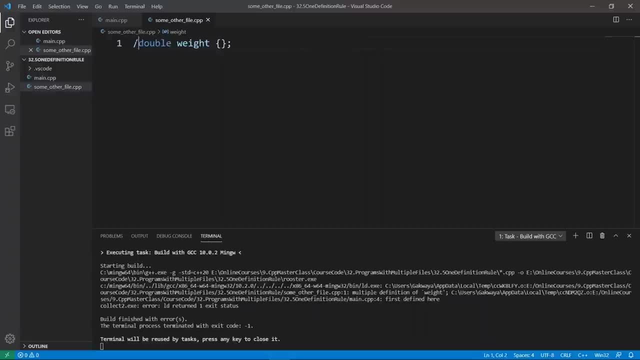 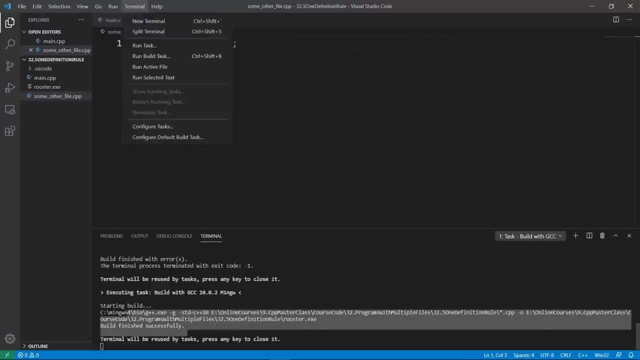 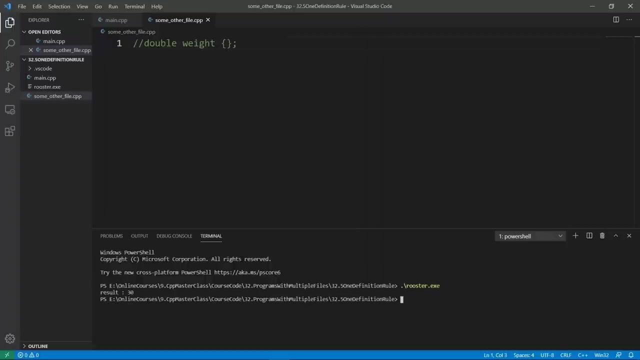 We have weight defined multiple times. We're going to comment out one definition for weight And we're going to build again. Now the build is good And we can run this program. We can kill our terminal here and bring up another one and run Rooster, You're going to see that the 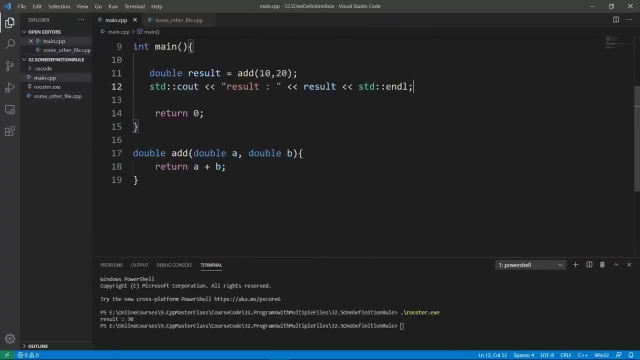 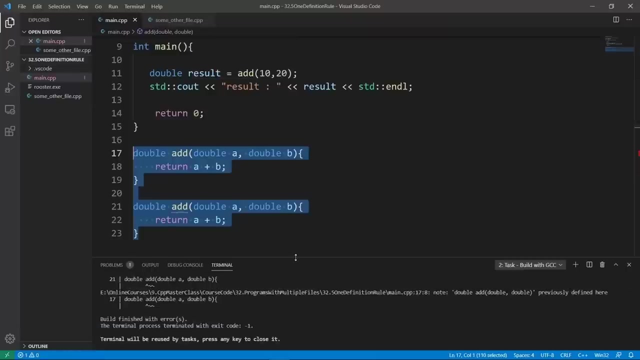 result is 30. And the program is working just fine. But if we set up another definition for add, even if we put this in the same file, we're going to get a problem because we are violating the one definition rule. Let's run again. You're going to see the problem here. We're going to see. 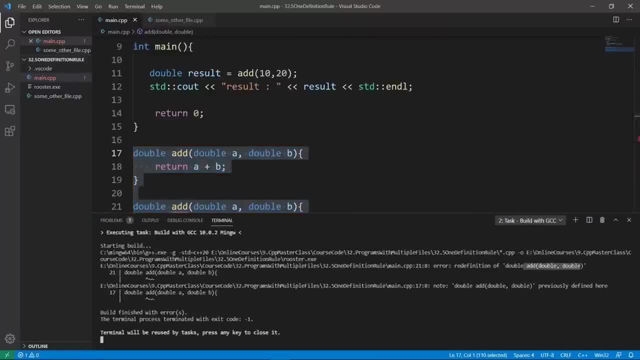 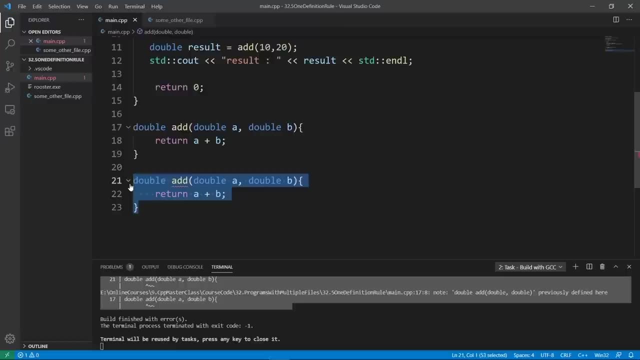 redefinition. Redefinition of the add function. This is not allowed. Your program is not going to compile. We see the compiler error here. Even if you put the definition in another file, that's not going to help. We're going to take this and put this in our some other file and try to compile. 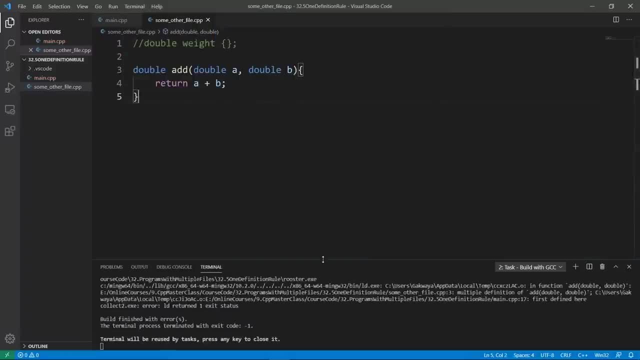 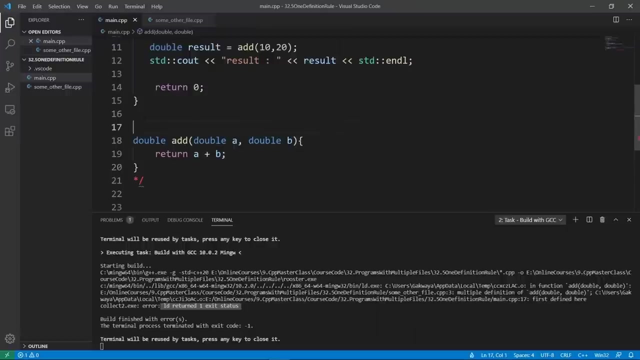 the program. We're going to get a linker error And it is going to say multiple definition of the add function And this is not allowed. This is a linker error in this time. If we comment out one definition, let's do that. We're going to comment out the one in the main function. This is going 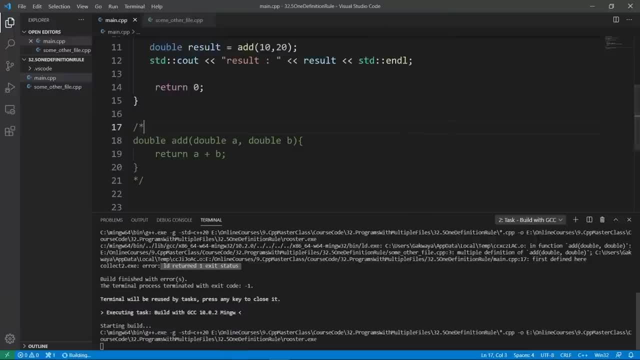 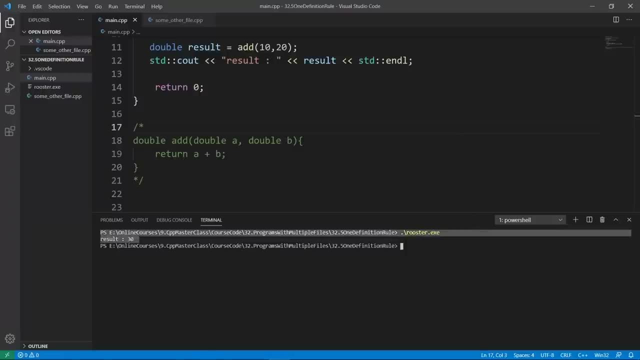 to work And we want to be violating the one definition rule. So this is good, The world is good, We can clear and run rooster. We're going to see our result here. So the one definition rule says you can't have multiple definitions for freestanding. 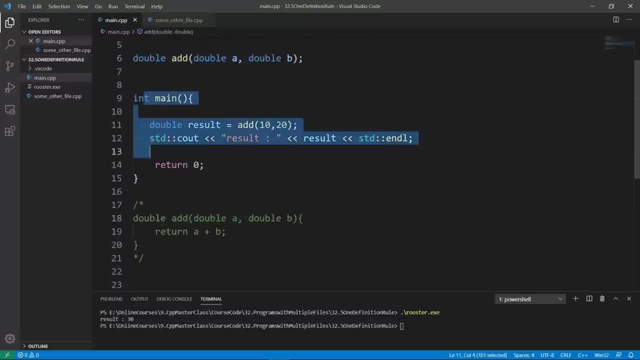 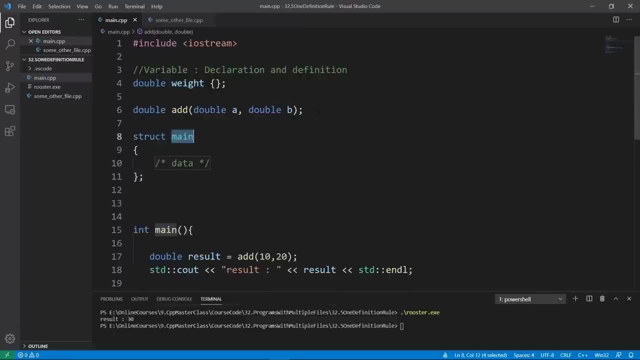 variables or even functions, And we saw that if you do that, you're going to get a compiler error. Let's look at this in the context of classes. We're going to do a class, We're going to say struct And we're going to call this point like we always do. Mostly, we're going to call this. 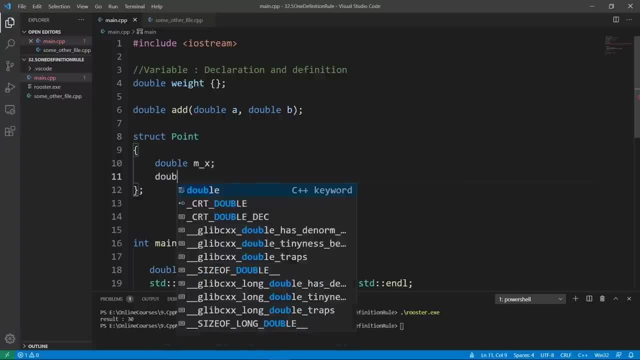 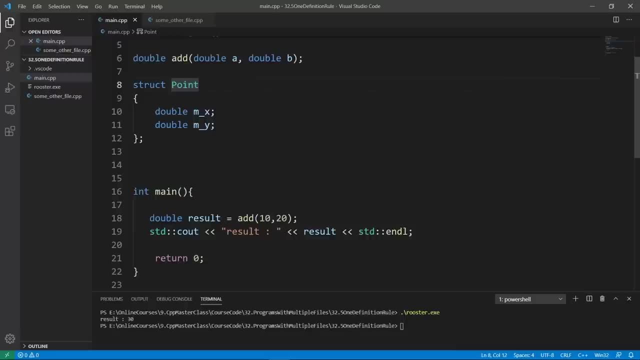 queue member variables. One is going to be MX, The other is going to be MY, And this is going to be our definition here. But what you're going to see is that it is possible to have multiple definitions for classes, For example, if we take this and have a copy of this in another file. 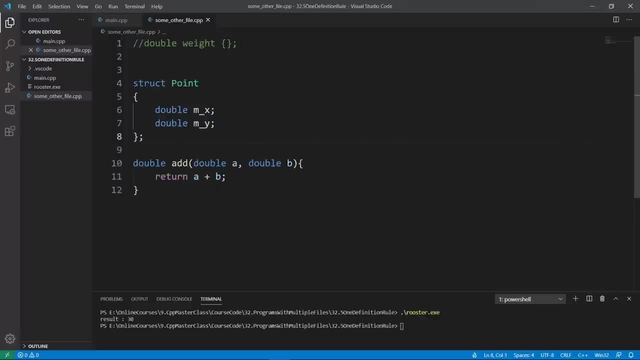 we're going to do that. We're going to declare this structure here And we're going to try and build this program. You're going to see that it is working. So we have multiple definitions of these guys. We can go in main, for example, and say point: 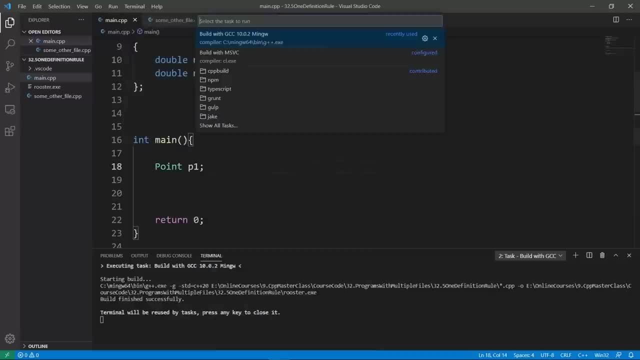 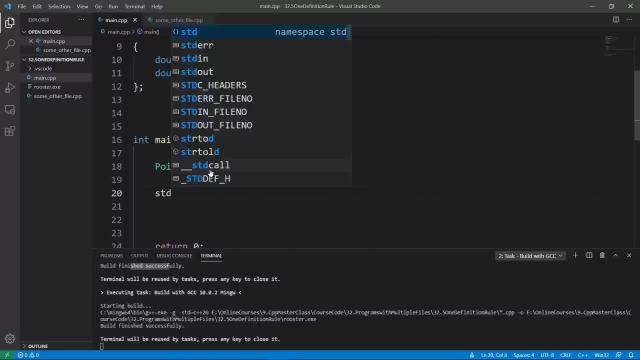 P1. And we can build and see that the program is going to work OK. So if you go in here, for example, and try to print STD, see our P1 and print X, we're going to do that. We're going to say P1- MX. We're going to be able to use this because 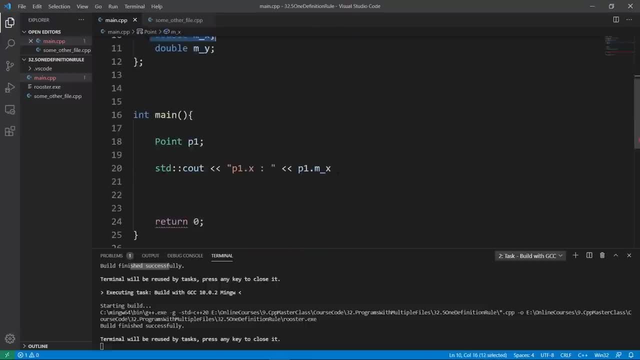 this is a struct. The member variables are public by default. We can do this, And we can say P1, Y is P1, Y MY, Let's do that. And we can say STD- NDL. What is the problem here? We need to. 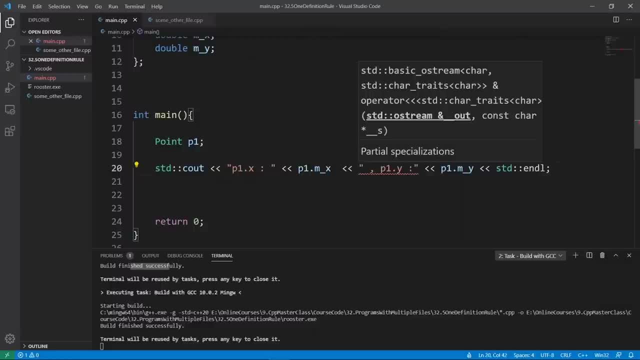 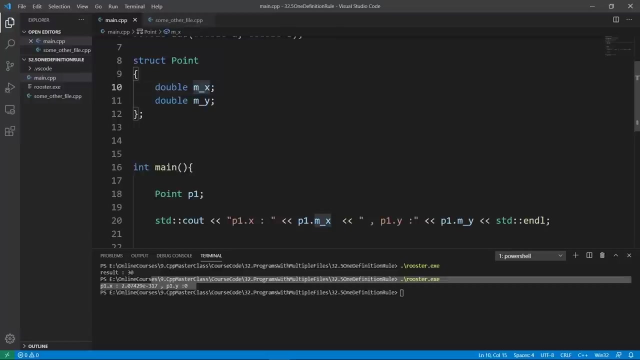 put our output stream operator. I think now the compiler is going to be happy And if we're built we're going to use GCC. We're going to see that if we run the program we're going to see our things here And we have some junk values inside because these things are not initialized. 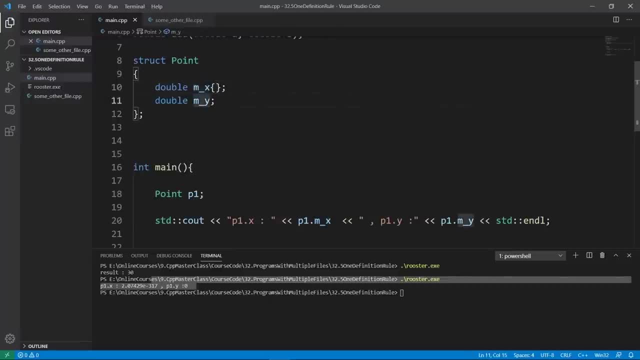 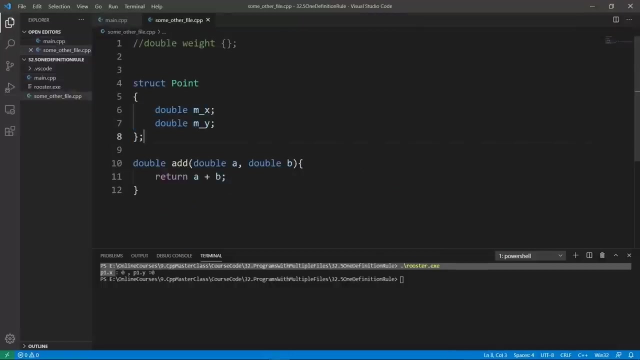 But if we initialize them to zero using a braced initialization here, we're going to build again And we should see zero inside. So let's clear and run rooster. Now we have zero in X and Y for our object here. This is working fine And we have multiple definitions for our class. But the definitions 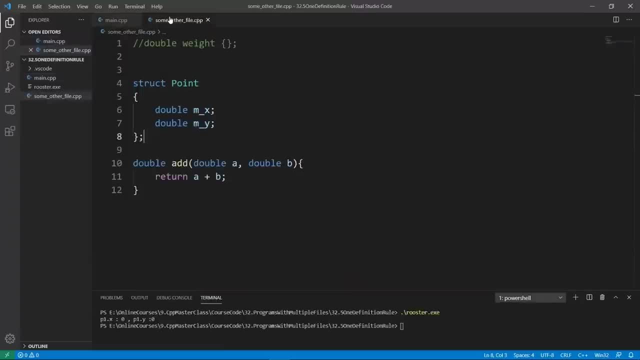 can't show up in a single translation unit. For example, if we took this definition here and brought that back in main and put that just below our struct here, if we try to build, the compiler is going to complain because now we have multiple. 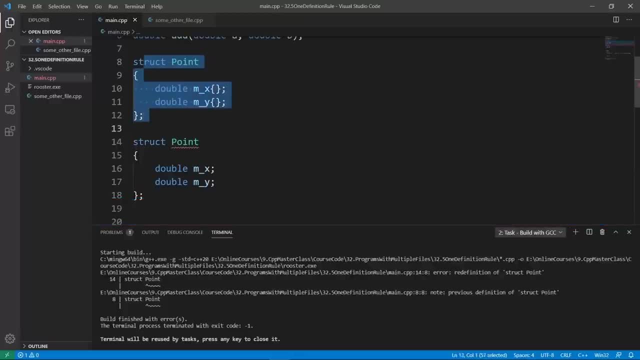 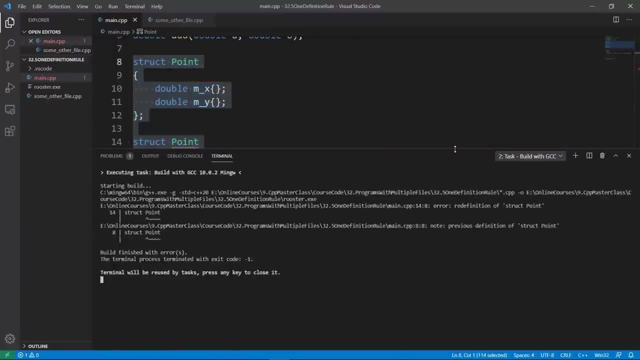 definitions for the same class in the same translation unit. For classes, we can have multiple definitions, but the definitions have to show up in different translation units, And that's what I want you to see here. So we have a redefinition of our point struct and it is not. 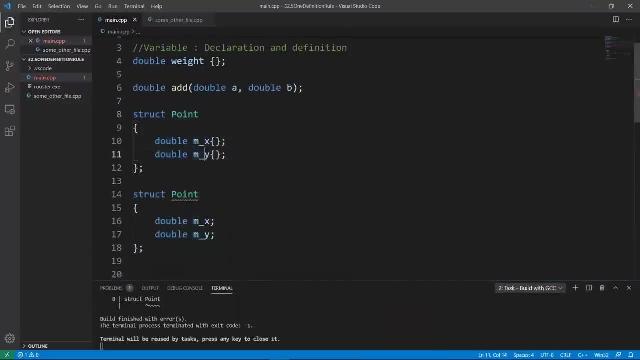 good, It is going to violate the one definition rule. Okay, now that you have seen this, we're going to use a margin graph here to show you what we can do with like this, And we also want to see this in the context of a class that also has some static member variables. We're going to take 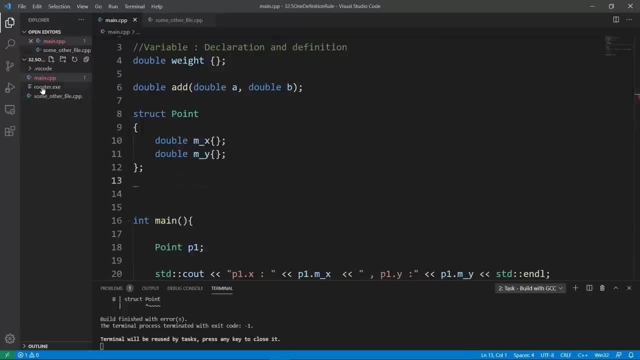 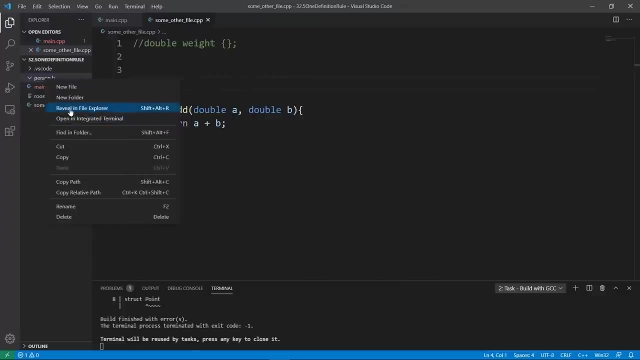 this out because we have already seen this and we're going to bring in our person class like we used in the last lecture. We're going to add in a new header file- it's going to be called person dot H And we're going to jump into. What did we do? is this a folder? Let's remove this. we. 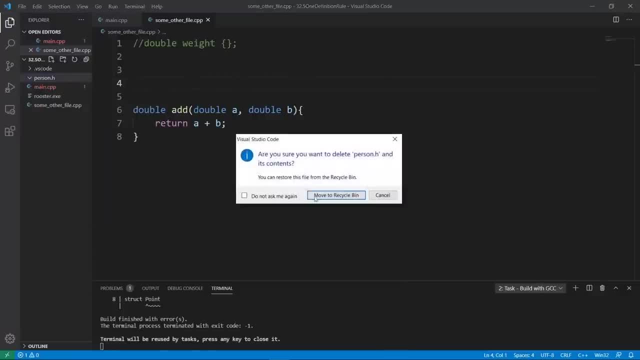 didn't want a folder. we're going to delete this folder. we don't want it and we're going to just add a file called personh. that's our file here and we're going to put in the content. the content is going to be our. 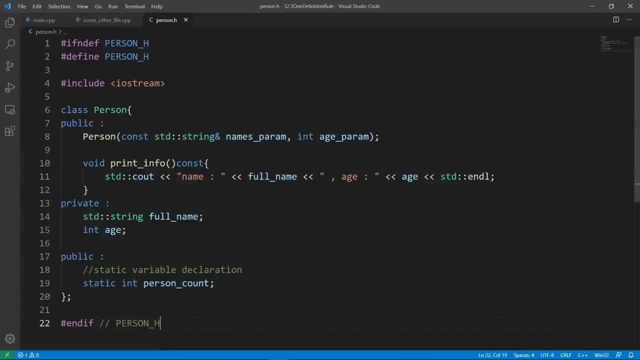 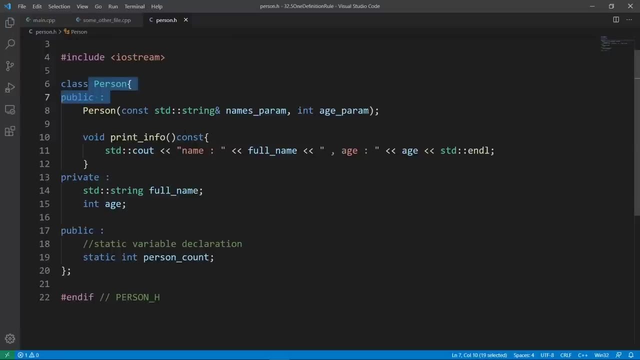 person class. let's close this so that you can see more of this class here. okay, so we have our person class here, we have our include guard, we have our person class definition, we have a constructor and we have a printable function. we have our member variables and down below here you see that we have 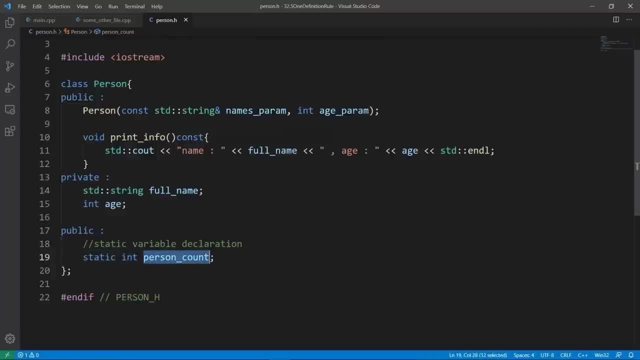 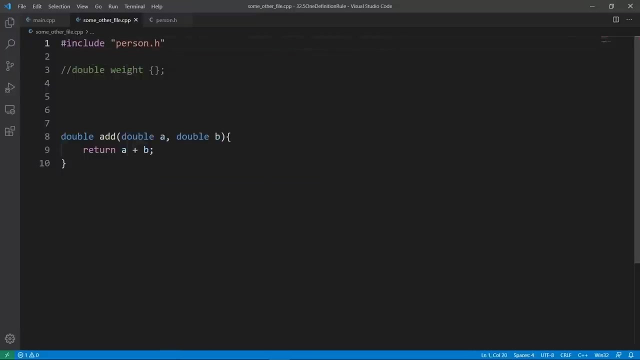 a static variable, which is person count. we need to put in the definition for these guys. so let's go down and do that. we're going to put in the definition for the person constructor. we're going to go on top here and include our person header file and we're going to put in place our constructor. 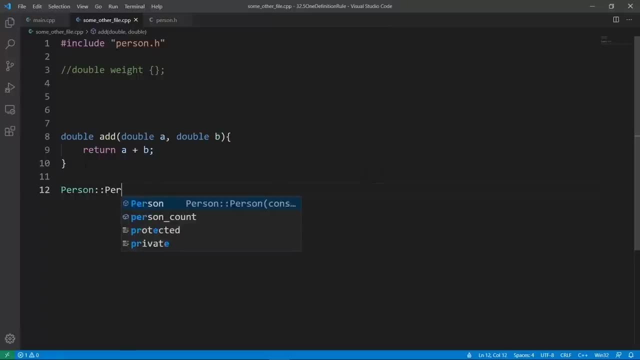 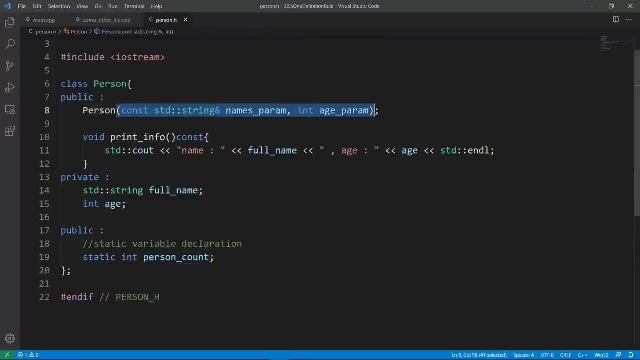 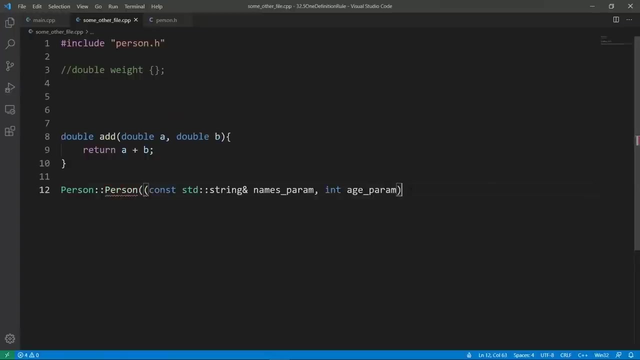 we can go down and do that. we can say person and say person, that's going to be our constructor. we're going to go back to the class and grab the parameters, because i don't want to type all these things, so let's do that. we're going to put them in. we are going to put in our initializer list. i think we should. 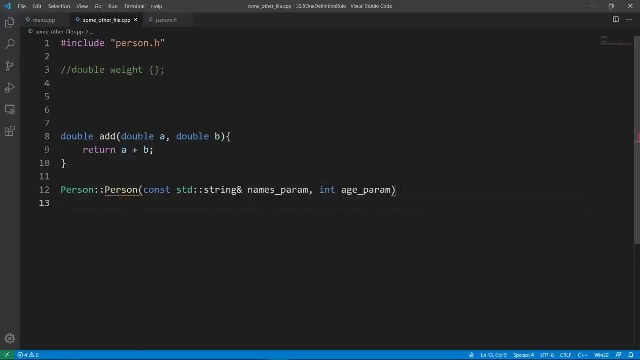 also delete a parenthesis here. we're going to go down and put in our initializer list. we're going to say full name, we're going to initialize this with name param, and we're going to also put in our age and we're going to initialize this with age param, the parameter we have from the function. 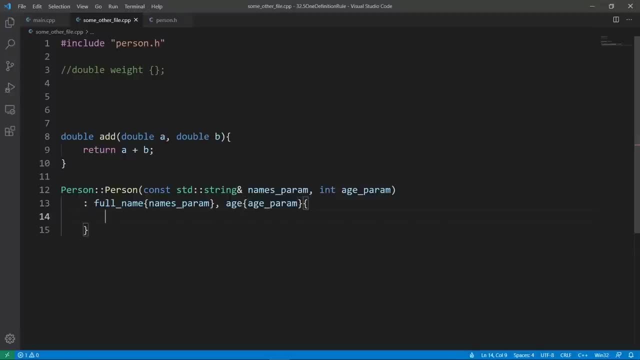 and this is going to be all inside the body. we're going to increment the static variable. we're going to say: increment person count. okay, and i'll select that here and this is going to be good. we also need to initialize our static variable. so we're going to say: int person, person count, let's do person. 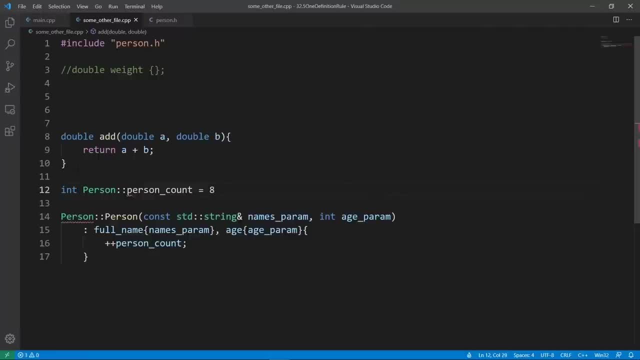 count and we're going to initialize this to maybe eight, like we did in the last lecture, and we're going to initialize this to maybe eight, like we did in the last lecture, and we're going to initialize this to maybe eight, like we did in the last lecture, and we're going to initialize this to maybe. 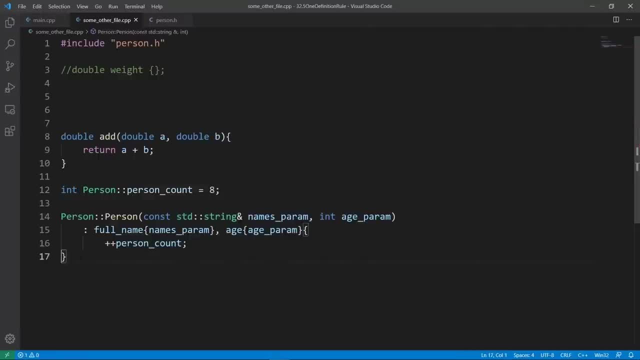 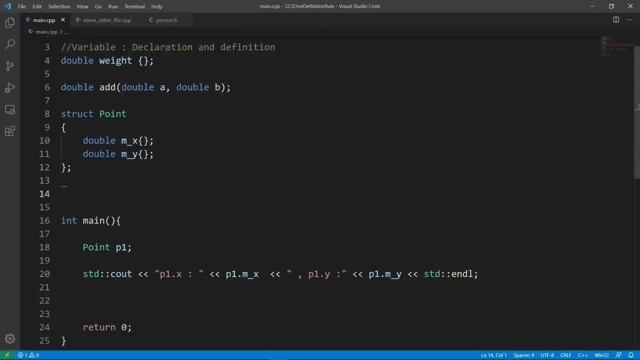 and this should be all we need here. so if we build and run this program- i think it's going to run- let's set up the main function here, and what problem do we have here? let's build and see. we're going to let the compiler figure this out. we're going to see that the build is good and we can. 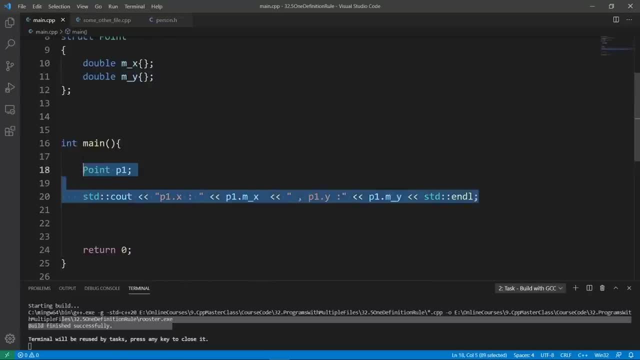 create person objects and really use them in our program. so let's come down here and delete whatever we had. we're going to include person and we're going to go down here and create a person object. we're going to say person p1 and we're going to specify the name to be jones- no, why not? and we're going to say that. 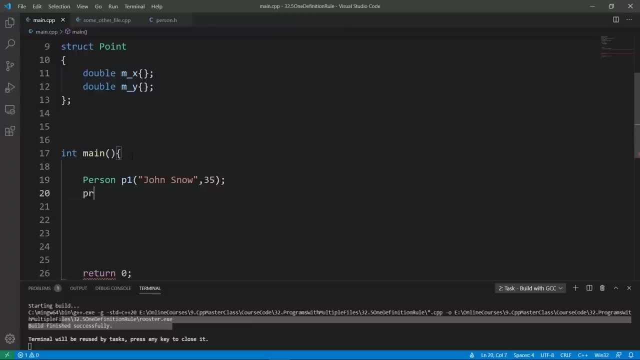 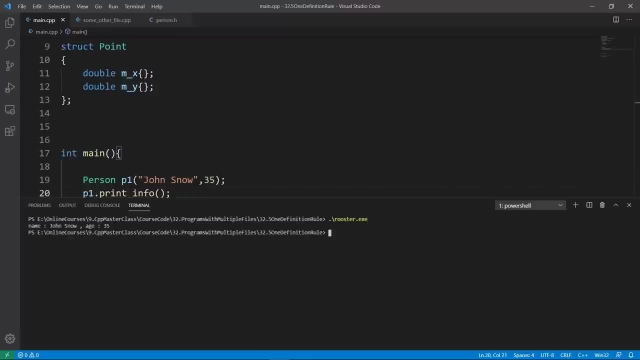 they are 35, why not? and we can print information about this person. we can say person printable and if we try to build this program, let's use gcc to do that. the build is going to be good. as you see, down here we can clear and run rooster. we're going to see jones. no, he is 35 years old, so this: 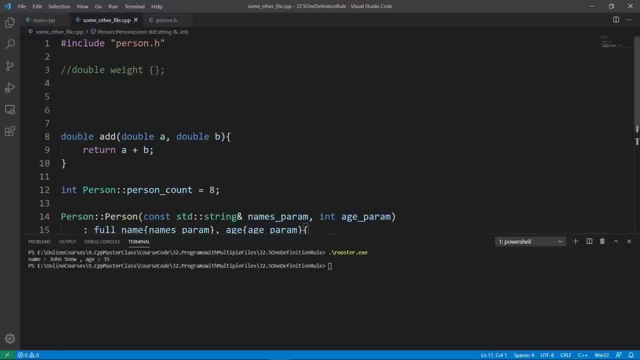 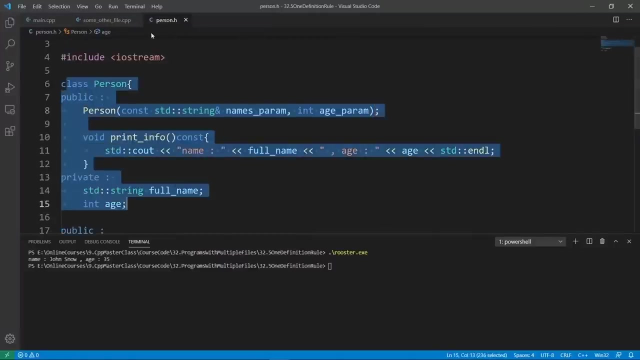 is working just fine. but we can't have multiple definitions for the same class in the same translation unit. here, for example, if we come in the main function, notice we are including person. so this is bringing in the definition for person we have in our personh. here, if we also try to declare another class, 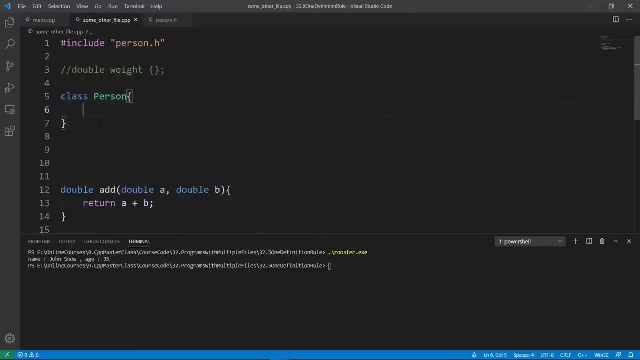 called person even if we don't put anything in. the compiler is going to complain because we have two definitions for the same name. we're going to say person and we're going to say person printable, which is person here. if we try to build, i think we are going to get a compiler error saying that. 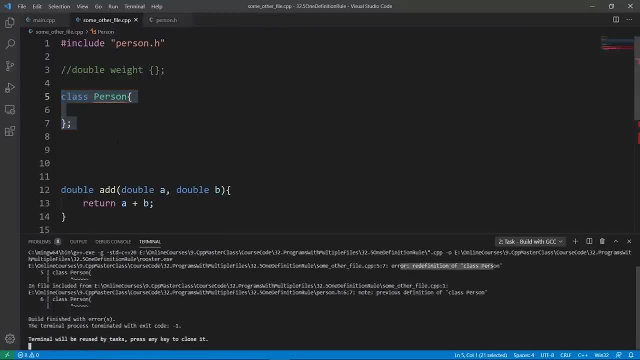 we have a definition. you see, we have a redefinition of person, so this is not allowed. we can't really do this. but notice that this person class is included both in some other file, which is a separate translation unit, and main. we have it included here, so it is really in a separate translation. 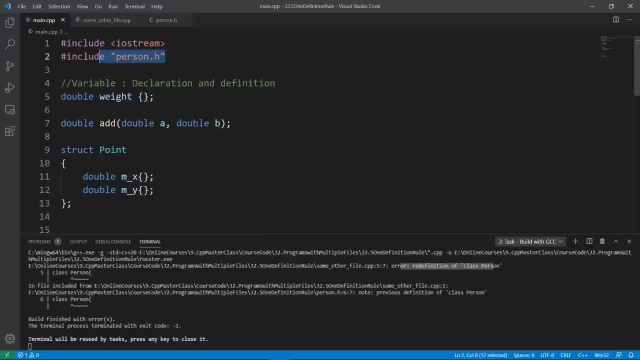 units. we have the definition for the class in separate translation units and we have the definition for the class in separate translation units and that's not a problem. but if you try and put the same definition multiple times in a single translation unit, you're going to get a problem and 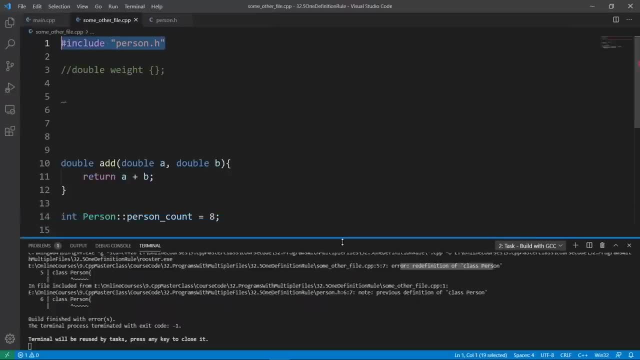 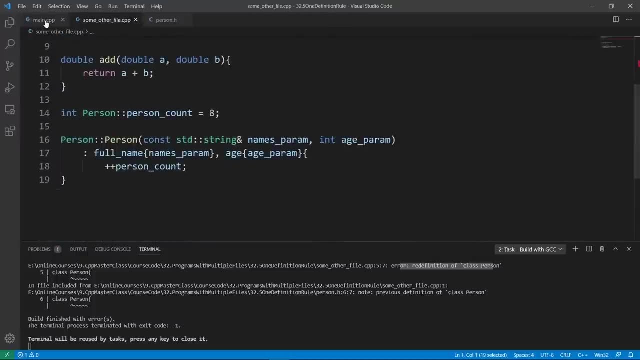 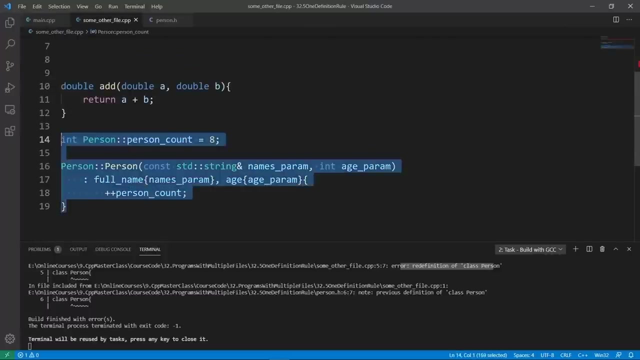 you need to be aware of that. what i want you to see right here is that you can't also have multiple definitions for your static variables and the member functions of your class. for example, if we grab what we have here and also put that in our main function, we can do that, and then we can also. 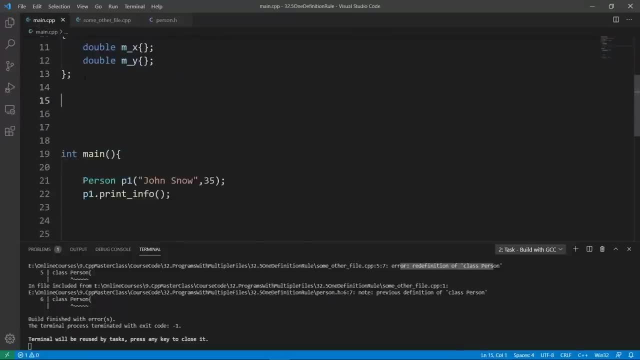 put that in our main function here and we're going to put the same definitions here. now we're going to have a problem because the linker is going to see two definitions for the static variable and the constructor for person here, and this is going to be a problem. you can't really do that. 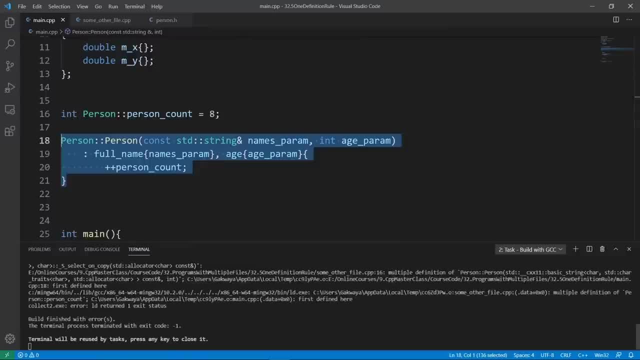 if we're built, we're going to see a problem. we're going to see that the problem is we have multiple definitions for the constructor and we have multiple definitions for person and we're going to have multiple definitions for person account, and this is not allowed. you can't really do that. 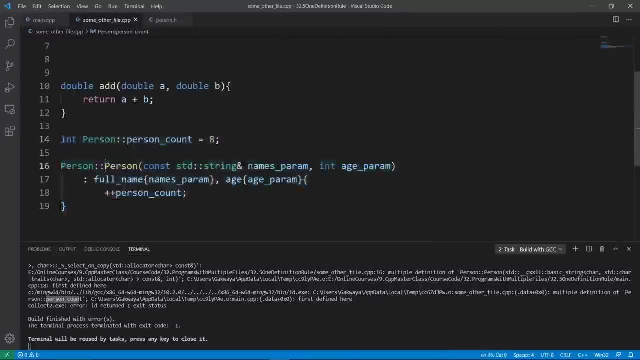 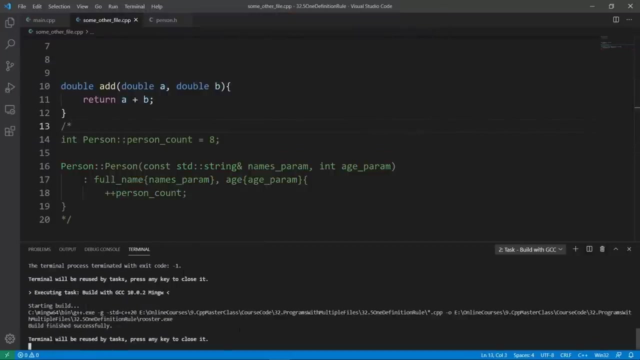 you can either remove the one from some other filecpp, for example. if we comment this out, let's do that- we can come on top here and comment this out and try to build the program. now the program is going to work because we have one definition for these guys. you see, the world is. 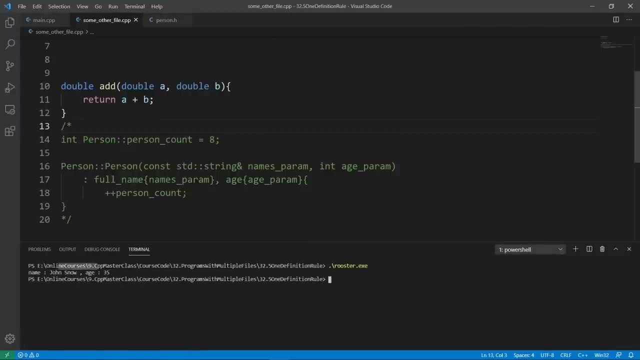 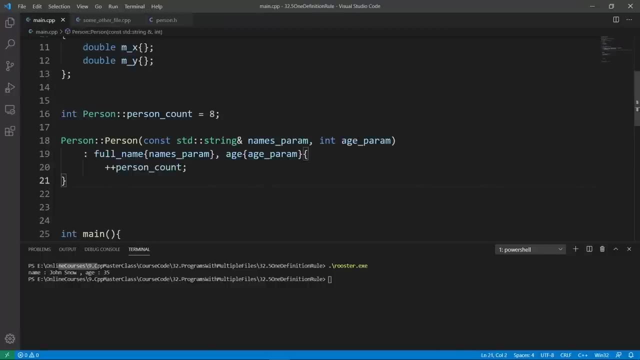 good, we can even run the program to show you that it works. or we can remove the one in the main cpp file and we can leave the one in the main cpp file and we can leave the one in the main cpp file. this alive. so let's go back in the cpp file, the main cpp file, i should say, and remove this. and if 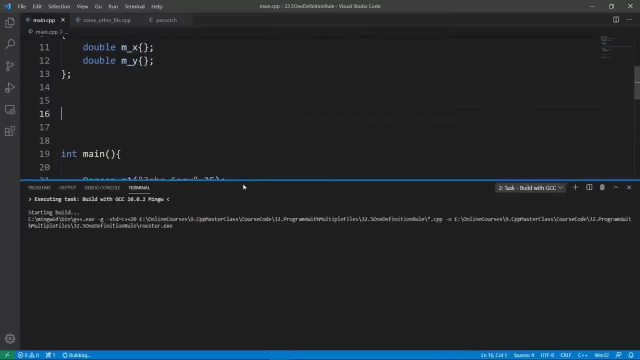 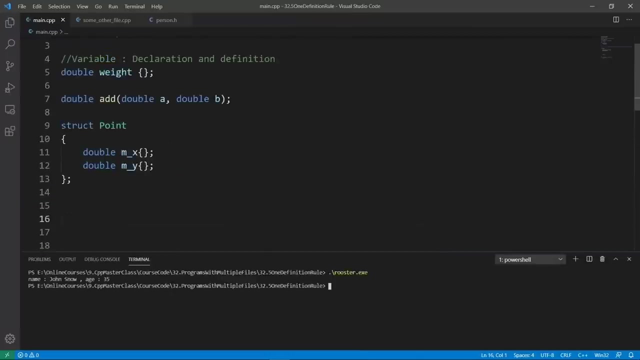 we're both. we're going to see that this is going to work and we are compliant with what the c++ standard expects us to do in our c++ programs. if we're around, we're going to see that this is going to work and this is really cool. this is really all i wanted you to see in this lecture, the one. 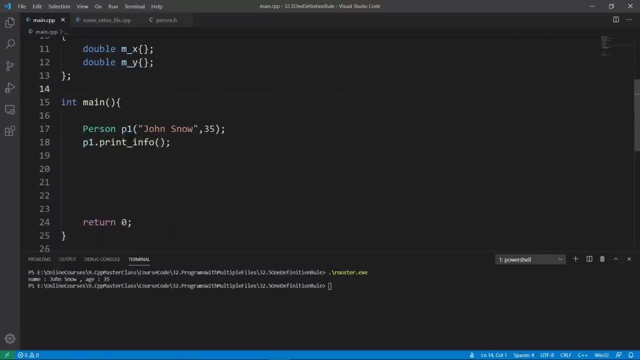 definition rule which says that you can't have multiple definitions for the constructor and for the same name in your entire c++ program, but for classes. we can violate this rule a little bit and make the same definition show up in multiple translation units. we are going to stop here in. 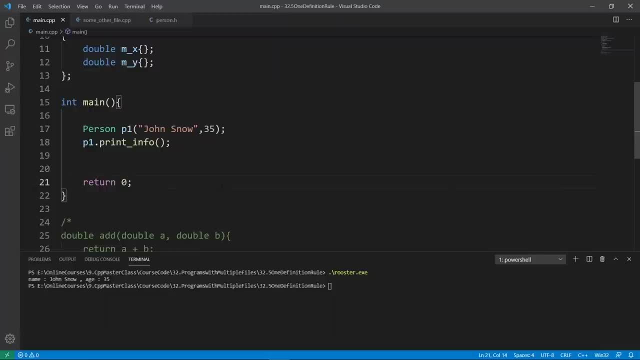 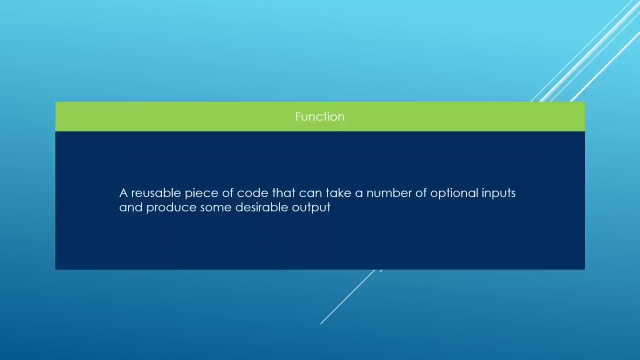 this lecture. in the next one we're going to learn about linkage. go ahead and finish up here and meet me there. in this lecture, we're going to learn about functions. a function is a reusable piece of code that you can use to create a function that you can use to create a function that you can use. 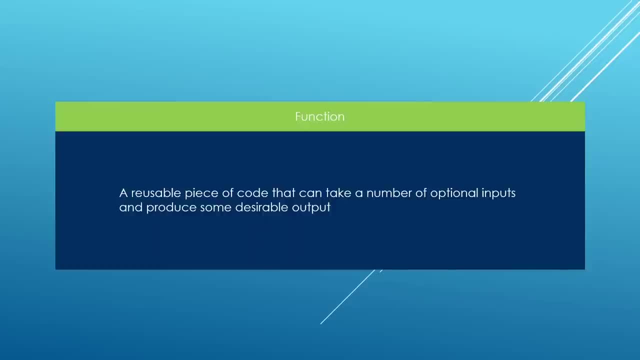 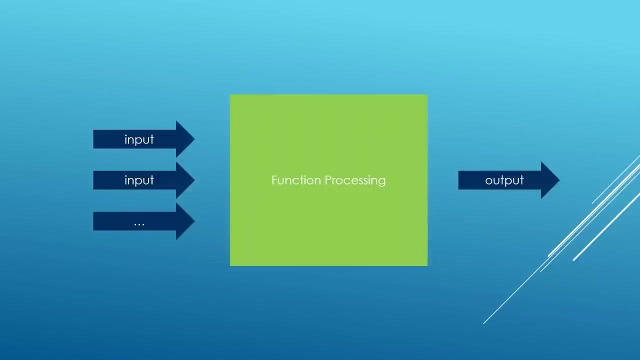 multiple times to do different things. it can take input and once it has input it can do some processing and when the processing is done, the function can optionally give you a reserve. you can think of a function as a machine which can take input and give you some output when you give. 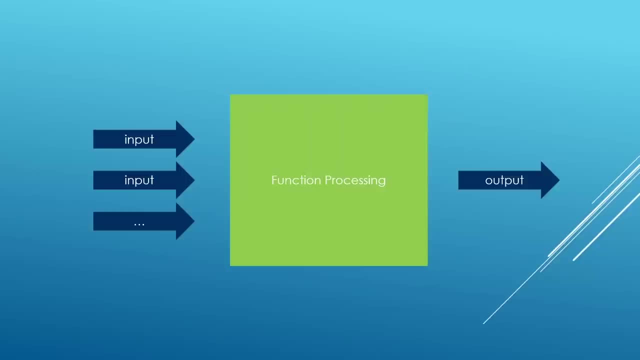 input to the machine. the machine is going to do some processing and then it's going to give you the output, and the output is going to be dependent on the input that you gave to the machine. this is really how a function works in c++, and once you have the machine set up, you can really reuse it. 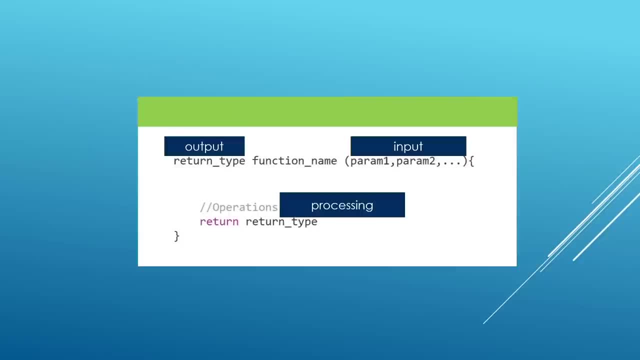 however many times you want. let's look at how a function looks in c++. the syntax is this: you first specify the return type, which may be and, double or whatever. after that, you're going to specify the function name, and after that you're going to have a pair of parentheses inside this: parentheses. 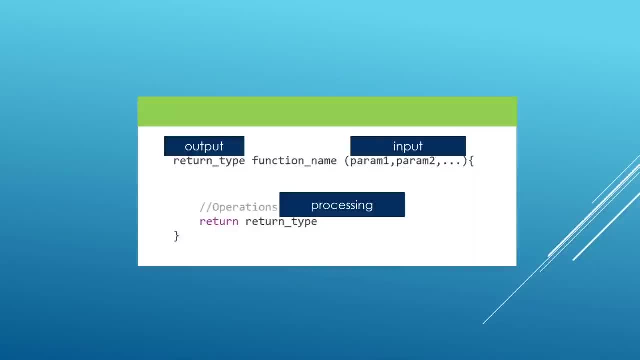 you're going to have your parameters, which is going to be a comma separated list of the events you pass to the function, and after all these parameters, you're going to have a pair of curly braces and inside those curly braces we're going to have the body of the function. we're going. 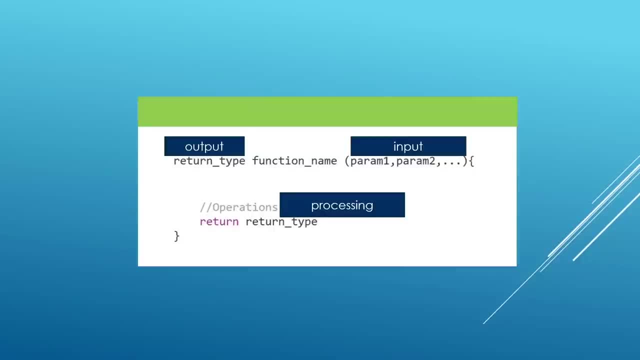 to be doing our processing in the body, and when the processing is done, we can get the result of the function through this return mechanism here. so if we want to get something out of the function, we have to return that thing and it is going to be visible to whoever. 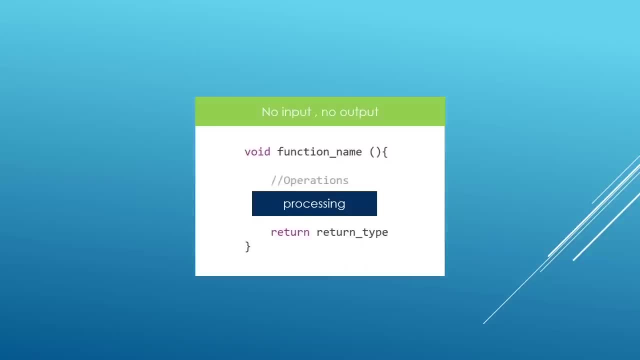 used this function. here is a simple example of a function with no input and output. the syntax is going to be: this void means that this function is not going to return anything, and you notice that our pair of parentheses is empty because we have no input in this function. we have our curly braces. 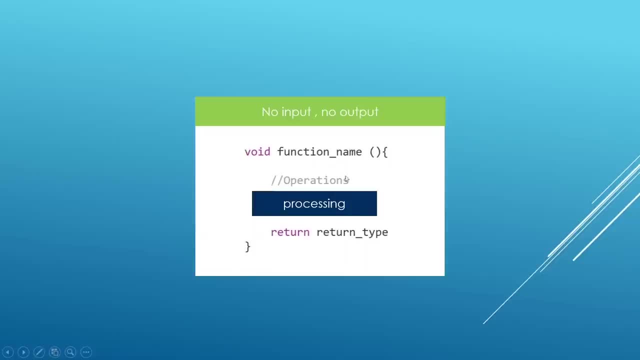 and inside these curly braces is going to be the body of this function. it's going to do some processing, and when processing is done we return out of this function. now remember that i said that this function doesn't return anything because it is of void type here. but we can return, and i'm going to show you the exact syntax of how you can do that. okay, so we? 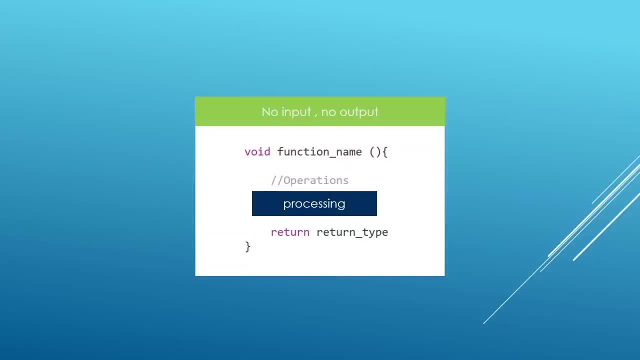 can have many functions in c++, but each function has to be unique, otherwise you're going to have problems in your c++ programs. a function is going to be unique based on its signature, and a signature is really a function name plus the function name of the function, name of the function. 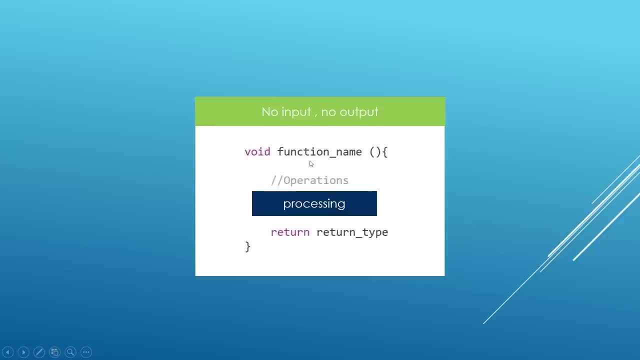 parameters. if we go back to our example here and try to figure out the signature of this function, it's going to be function name and plus the parameters, and you see that we have no parameters in here. so this signature is going to uniquely identify this function in our c++ program. if we 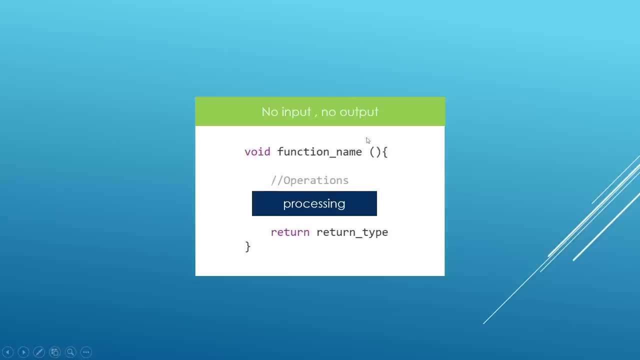 set up another function that has this same function name and doesn't take any parameter, we're going to have problems, even if we happen to have a different return value for the function. and don't worry if this is not making sense yet- we will see a lot of examples. 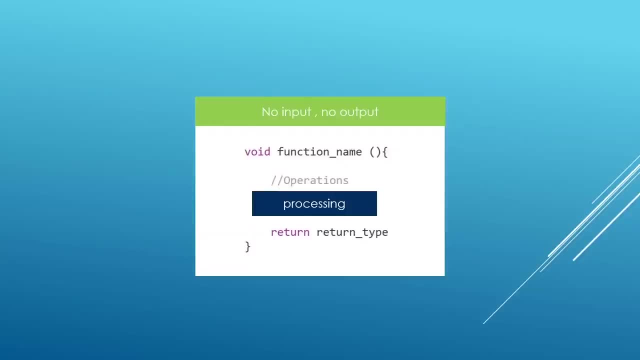 and i am sure by the time we are done with this lecture, you'll be a master at using functions. okay, now that we have seen how we can declare or define a function in c++, let's see how we can use the function. and when you call a function, in most cases you will want to get something out of that. 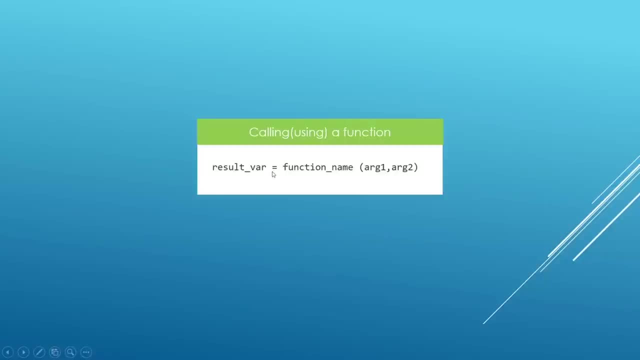 function. so suppose here, resort var is a variable that is going to catch the result of the function and we're going to call the function with a syntax like this: we're going to say the function name, we're going to put our pair of parentheses here and we are going to pass. 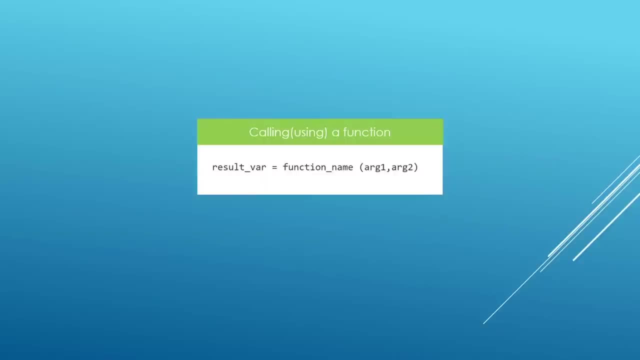 in the arguments or the values of our parameters. this is the syntax. it is going to call the function and the result of the function is going to be assigned to this result var variable of ours. here is how you can call a function that doesn't take any parameter: the parameter list. 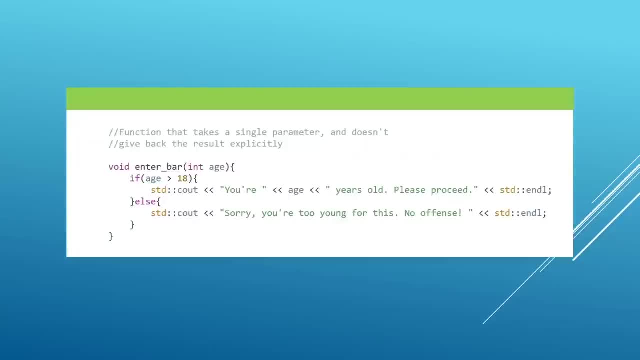 is basically going to be empty. and now we're going to look at a few examples of how you can really declare functions in your c++ program. for example, here we have a function called into bar. it doesn't return anything, so we can't catch the result of this function, and it's going to have one. 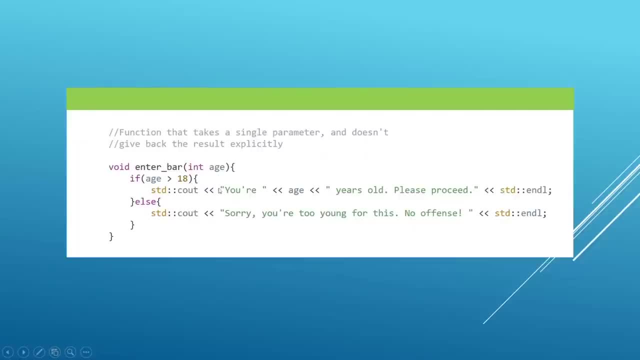 input in the form of an integer. so the parameter is called h here. it's an integer and inside the function we are going to test if somebody is old enough to enter a bar. so we do a test to see if the age is greater than 18. if it is, we're going to tell them. 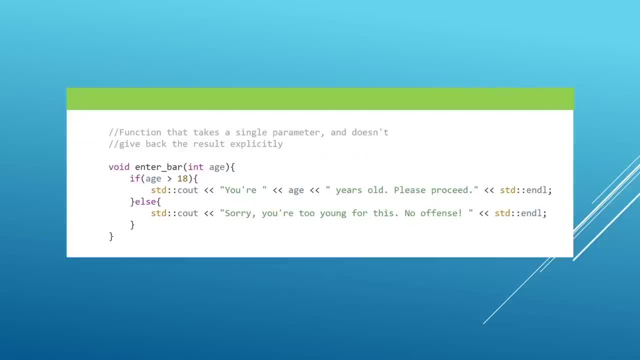 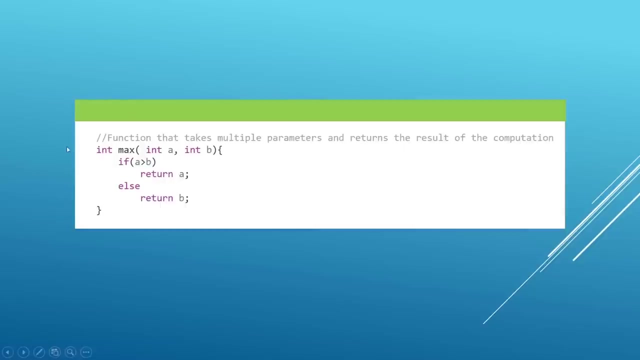 please proceed. if the age is not greater than 18, we're going to tell them you cannot enter. this is an example of a function you can set up in your c++ programs. here is another function that is going to compute the maximum between two numbers. it is going to give us a result, so the 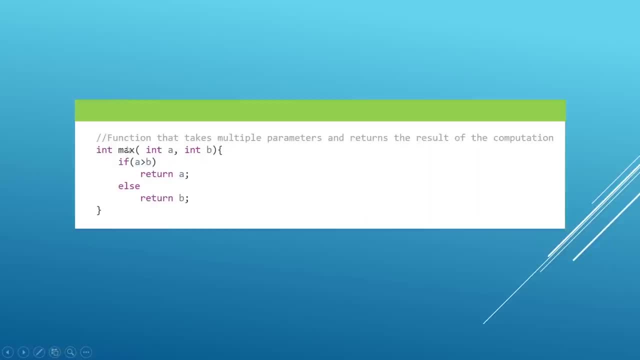 return value is an integer. here, the function name is max and we're going to put in our list of parameters. and again, these are the parameters when you are defining your function. this comma separated list of things we have in this parenthesis are called parameters, and when you 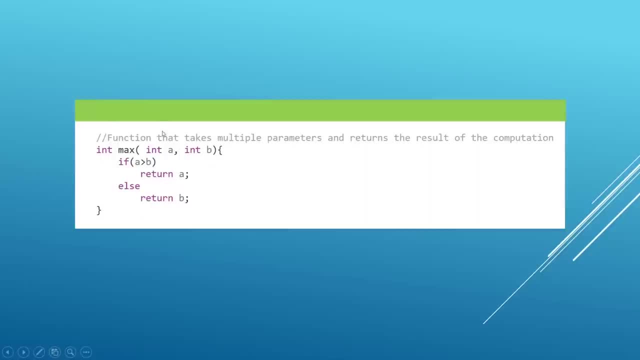 call the function. the values that you pass in the places of these parameters are called arguments. so these are a few terms that can really throw you off and I just want you to be super clear about these things. once we have the signature of the function set up, we 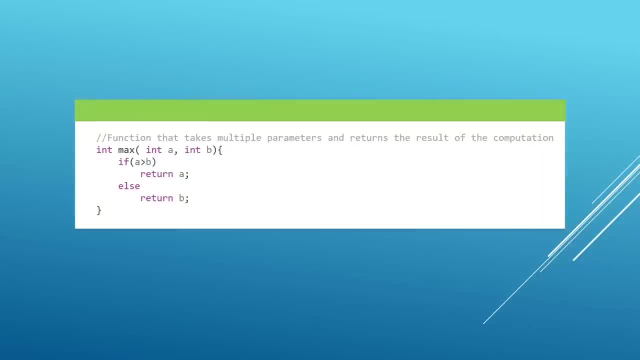 are going to put in the body and we do whatever we want this function to do. so we're going to say if a is greater than b, then a must be the maximum. we're going to send it that back to whoever called this function. or in other words, we're going to return a and if a is not greater than b, then b. 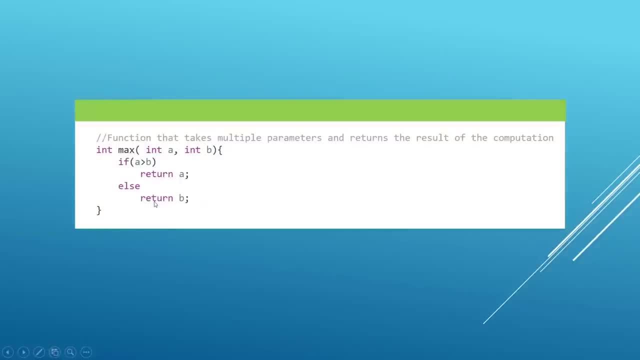 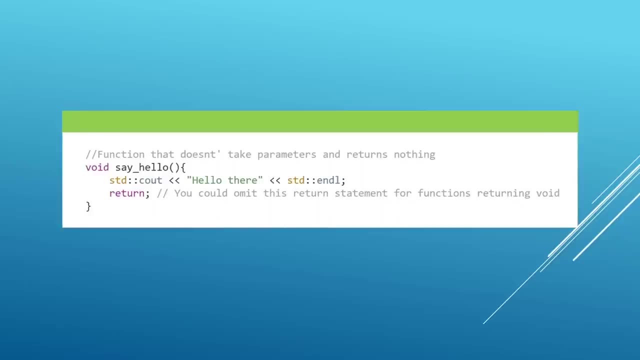 must be the maximum and we're going to return it. that's what we're saying here. here is another example of a function that doesn't have any output and doesn't take any input. it doesn't return anything because the return type is void and it doesn't take any input because the parameter list here. 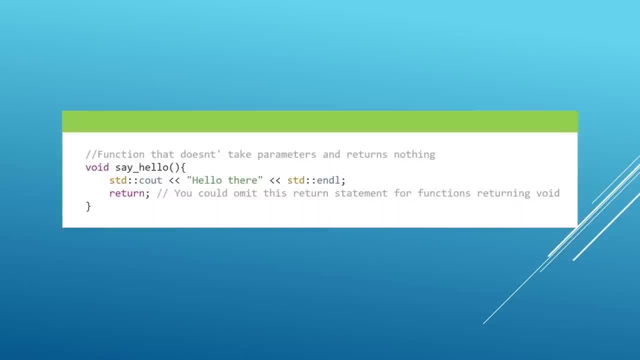 is empty and the body of the function. we're just going to greet somebody and tell them hello there and we're going to return out of the function. notice that for a void function we can either omit the return statement here or we can just put it in like this: say return and the semicolon. 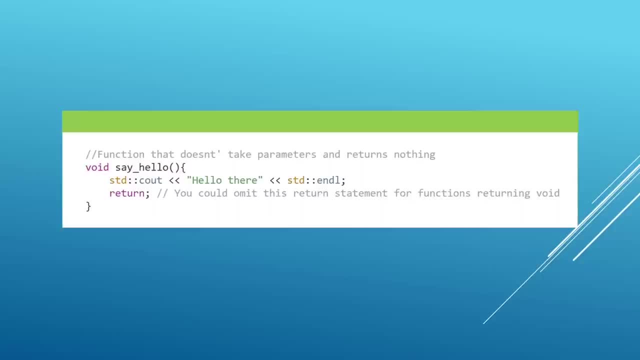 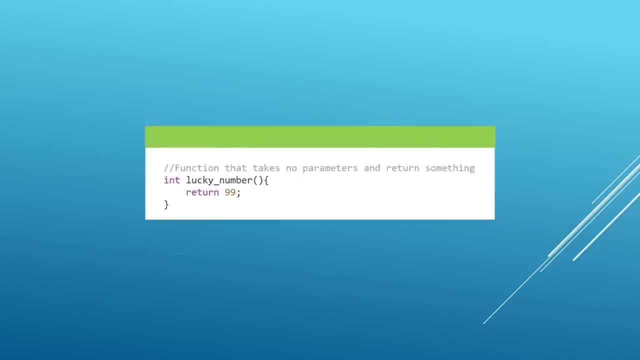 and whatever C plus plus compiler you are using is going to accept this as valid C plus plus syntax. here is another example of a function that returns something but doesn't take any input. the return value is going to be an integer, but we don't need to pass something to. 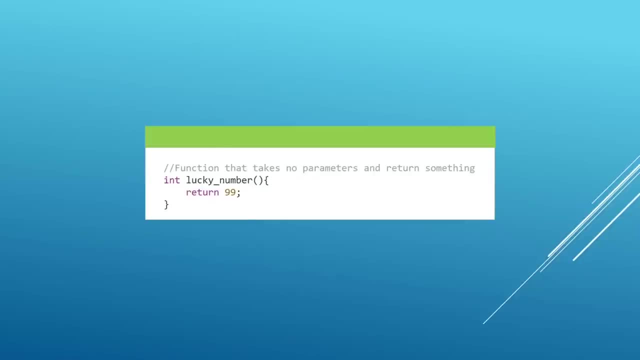 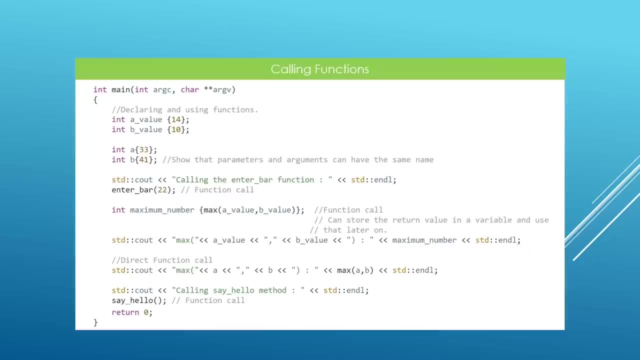 this function. when we call it, it's just going to give us output. we can call it and get our lucky number and use that however we want in our C plus plus application. I think we have seen a lot of examples of how we can set up functions. now let's see how we can call this function. 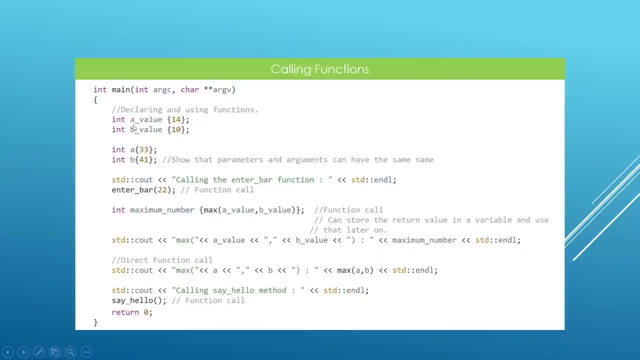 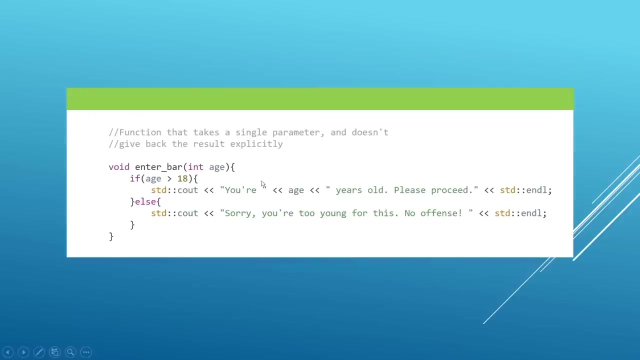 here is a simple C plus plus program. in the main function we just set up a few variables- a value B, value a and B here- and we use those variables to call functions. remember we set up an inter bar function. the function looked like this and it was testing to see if somebody's age was greater than. 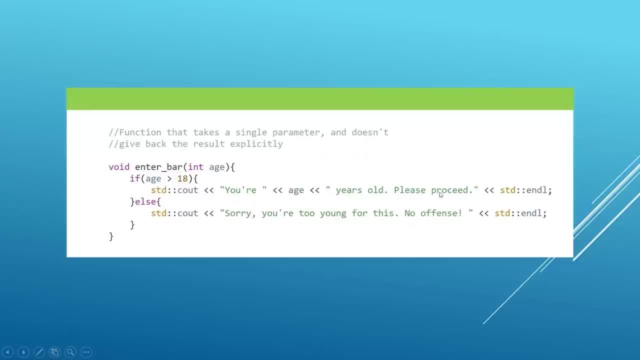 18.. if the edge is greater than 18, they are going to enter the bar. if the edge is not greater than 18, we won't let them in. the function takes the input but it doesn't return anything. so we can call this function like we do here and say into: 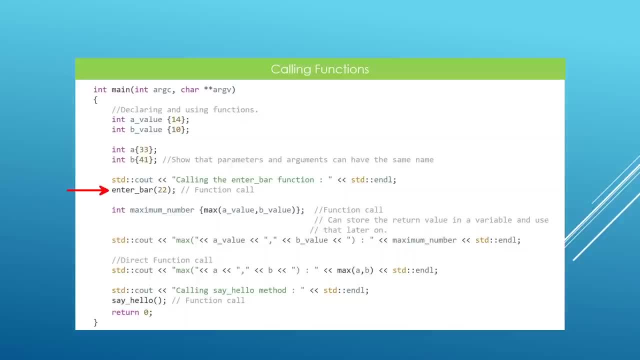 bar and you notice that we're not catching something out of this function. we're just going to call it and we're going to give it input, which is 22 here, and the function is going to do its thing. so it's going to let us in because our age is greater than 18.. down here you see, we are calling. 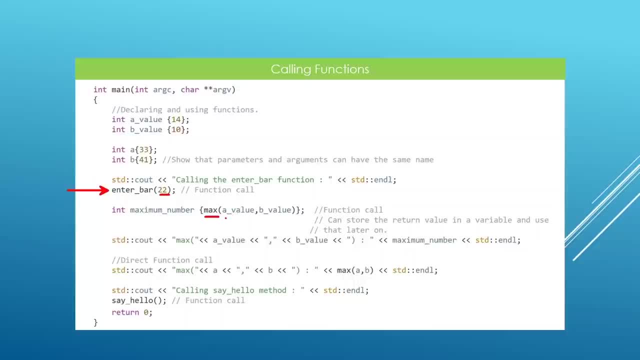 the Max function. here we are giving it two inputs, a value and a value, and it's going to return something, and the return value of this function is going to be used to initialize this maximum number variable here this is what we are doing. if we go down, we 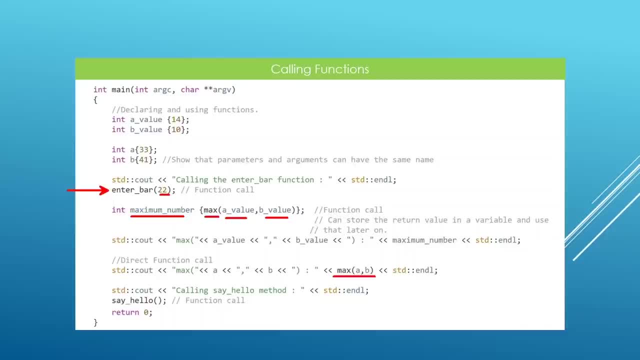 see that we can call the maximum function directly and use its return value in an std c out statement here and this is going to print out the maximum between a and b and down. here you see, we have the function say hello, which is going to just greet somebody and not 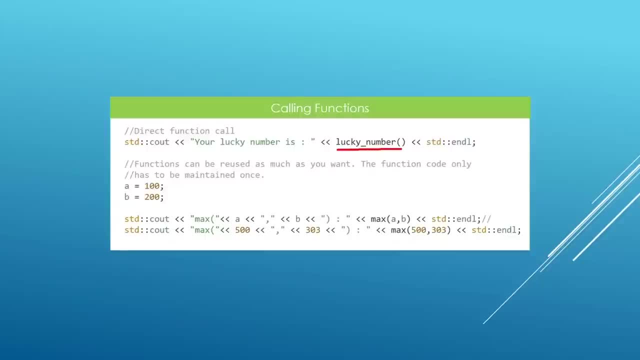 return anything. here is another example of how you can call the lucky number. you say lucky number, you pass a pair of parentheses and this is going to return the lucky number and print it out in this stdc out statement here down here. we set up a few variables, a and b, and we are going to use them to 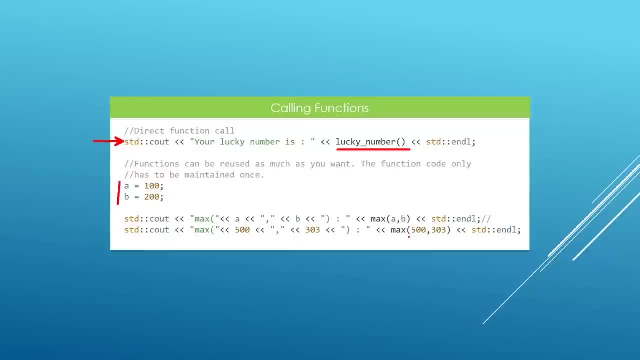 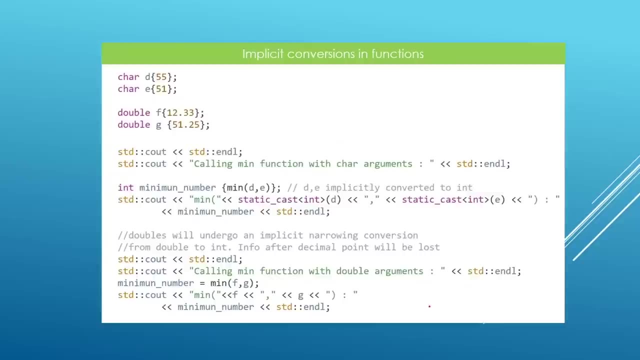 call the maximum functions. you see, we call Max a, b or we can even pass in number literals, like we are doing down here. what I want you to be careful about is implicit conversions. that might happen when you are calling your functions. suppose we have a minimum function, like we see here, which is going to be taking in. 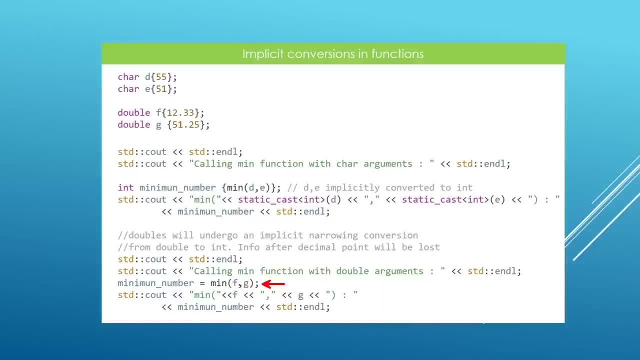 integer parameters. but here we are calling the function with F and G, which happen to be of double type, like we see on top here. so what is going to happen is the compiler is going to notice that what you are passing again is not really what the function takes. but 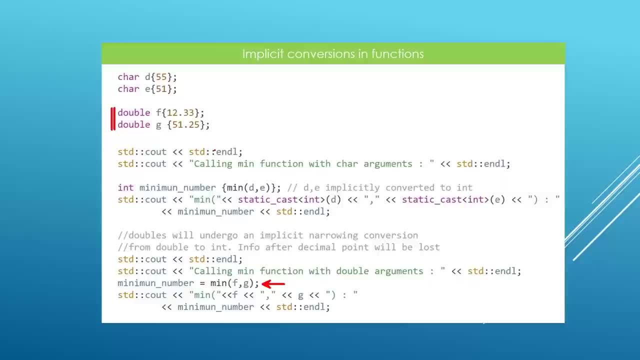 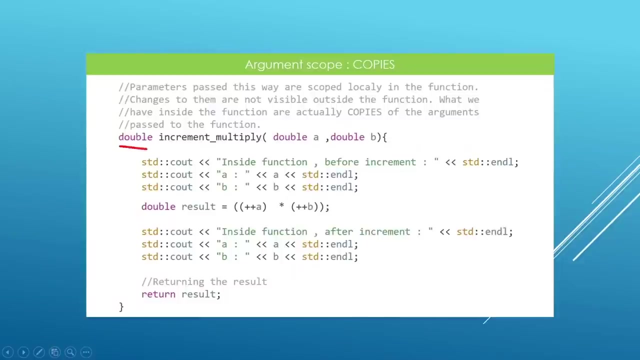 the compiler knows that it can insert a transformation from double to integer, and it is going to do that without your involvement. so be really careful about implicit conversions and make sure they are working to your advantage, otherwise you're going to have really hard to debug problems in your C++ programs. one other thing I want you to be aware of is that if we 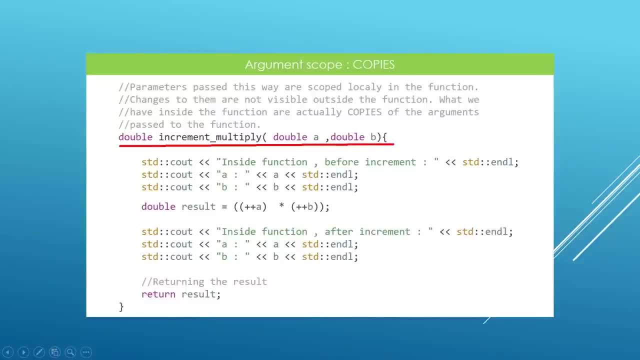 have a function set up like this, this function is going to be taking parameters as copies. so if you have two variables, for example C and D, and you call this function with those two variables, you're not going to be manipulating those two variables. what you will be working with inside the body of this function are going to be copies of the parameters that you 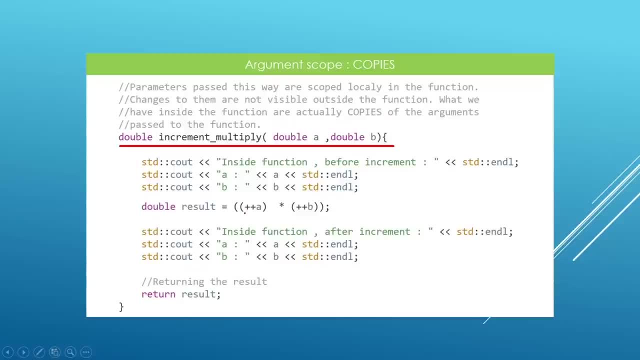 passed in here. so if, for example, you happen to increment either of the parameters- for example, here we increment a and we increment B- the changes we make here inside the body of the function are just going to be affecting copies we have inside the function here and these copies are going to die the moment we 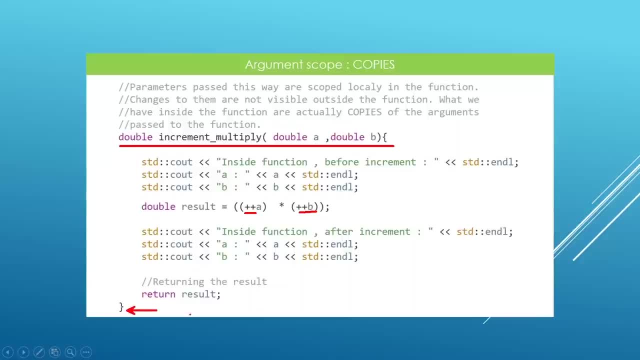 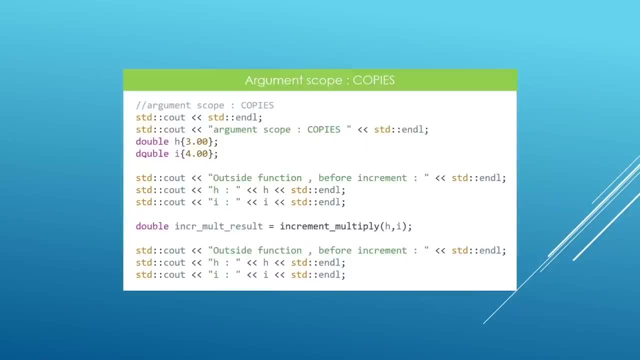 hit the end of this function here. this is something I want you to be aware of and we will play with that in more detail when we hit Visual Studio code in a minute. here is a simple example of how you can call that function. we have two variables, H and I, and we are going to print them out after. 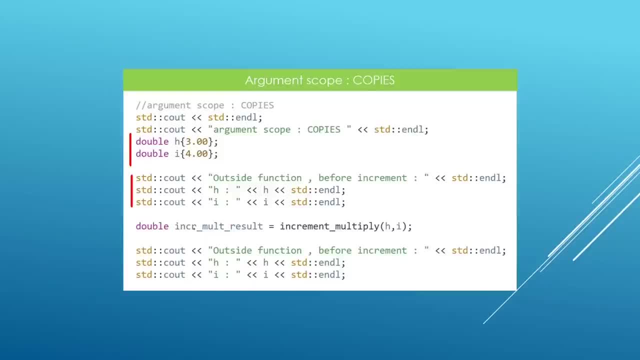 that we're going to call the function, we're going to store the result back in ink malt thirties, but the important thing is that we call the function here with H and I remember in the body of the function we are incrementing h and i as arguments, but the changes we do inside 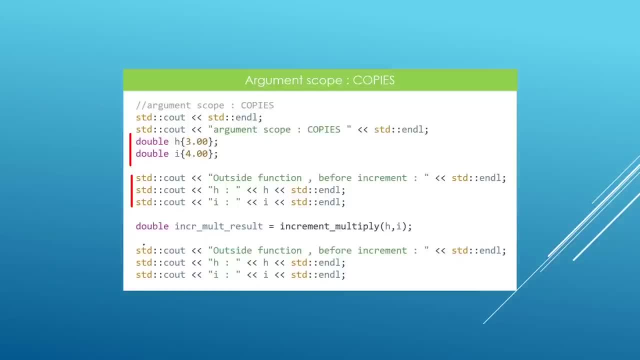 of the body of the function are not going to be visible when the function returns. if we print H and I here, we're just going to see the same thing we saw before we called the function. I realized this is a lot of information to take in. now we are going to head over to 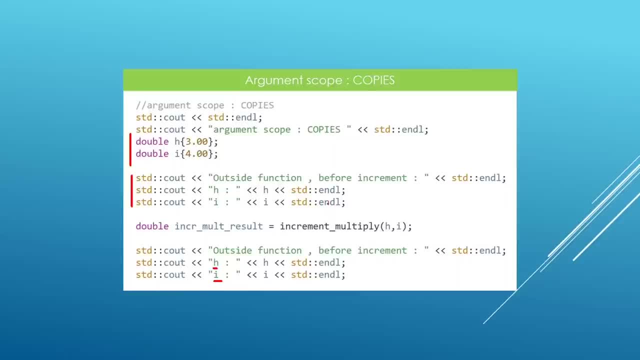 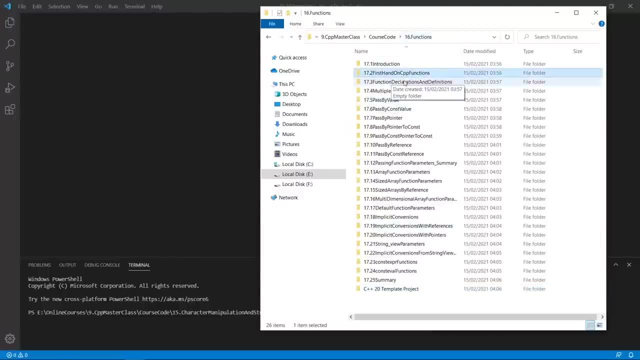 Visual Studio Code and actually play with this step-by-step. Okay, here we are in our working directory. The chapter is on functions. The current lecture is first-hand on functions. We are going to grab our template files, like we always do, We're going to put this in and we are going to open this in Visual Studio Code. 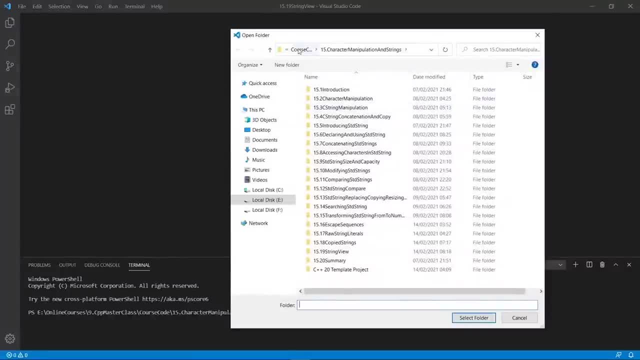 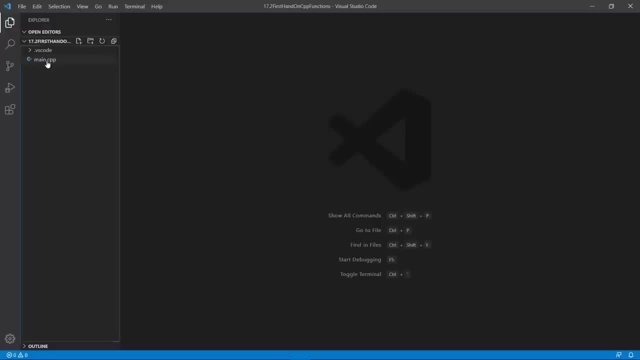 Let's open the folder and we are going to go in the correct chapter and choose first-hand on functions here. This is what we want to open And we are going to open our main CPP file and clean it up a little bit And the first thing we want to do is to set up a function that takes a single parameter. 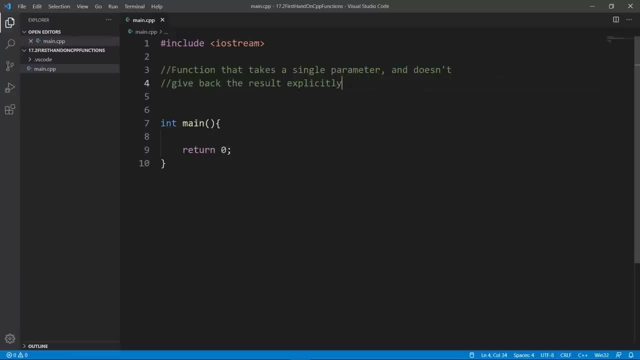 and doesn't give back any result, So the function is going to be interbore. We have seen that The function is not going to return anything, So it's going to be void. Its return type is going to be void. The name of the function is going to be interbore. 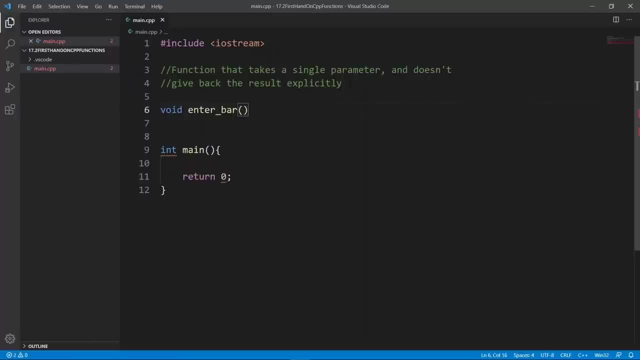 And what we want to pass in here is a variable to represent the age of somebody, And we know that the age can really not be negative. So it is advised to at least use an unsigned integer type. So we're going to use unsigned int. 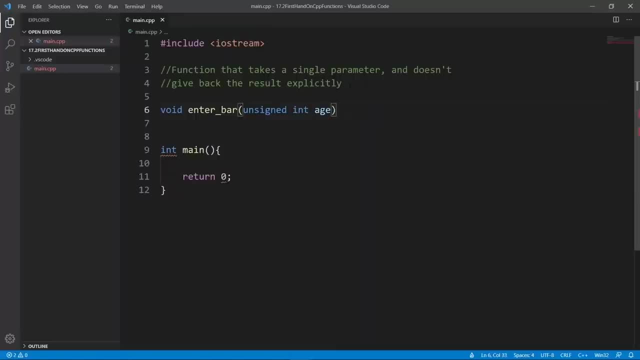 And the parameter name is going to be called age. Once we have our parameter list, we're going to put in the function body And remember, the function body is going to live within these two curly braces. Now, this is a valid C++ function. 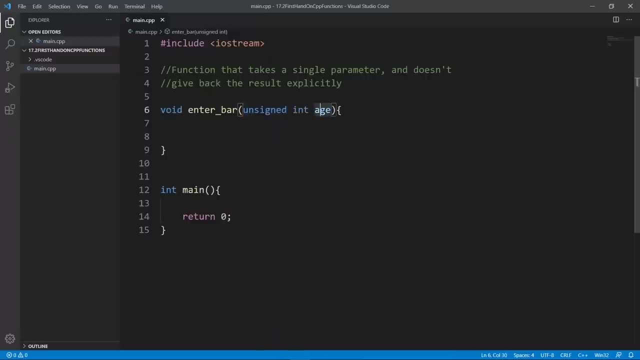 It's not going to return anything. It's going to take a single parameter whose type is unsigned int. Its name is interbore. We can get inside the function and actually do whatever it is we want to do. So once we go in, we're going to test and see if the age is greater than 18.. 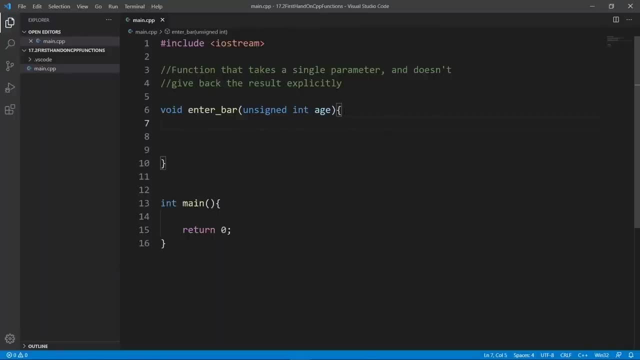 Do something. If the age is not greater than 18, we're going to do something else. Let's do that. We're going to say if age is greater than 18.. We're going to tell them The age and tell them that they can actually go in. 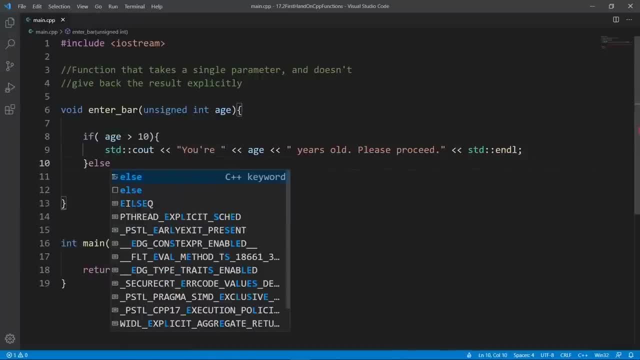 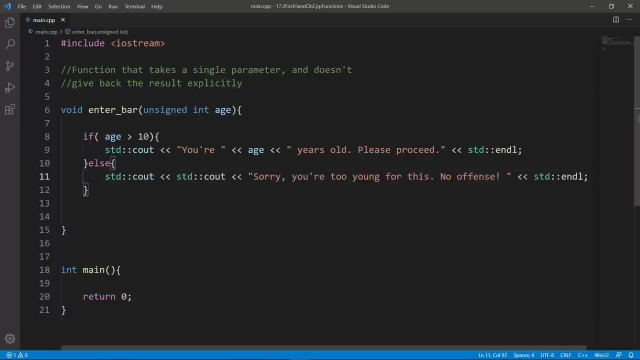 This is logical And we're going to say else. And in the body of this else block, we're going to say something else. We're going to tell them: sorry, you are too young for this, And we are going to get out of this block here. 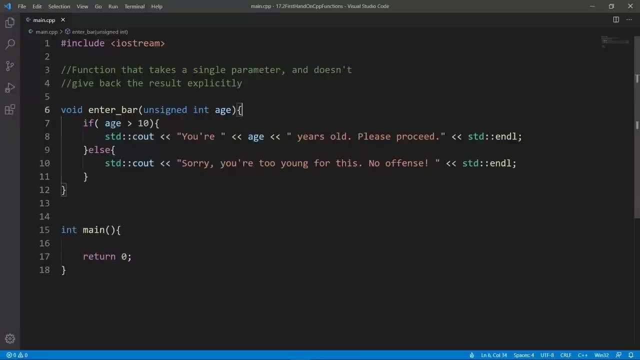 And this is really our function. Again, let's try to analyze the syntax. here We have the return type. This is required in C++. If you don't put it in, you're going to get a Compile Error because you can't have a function without a return type in C++. 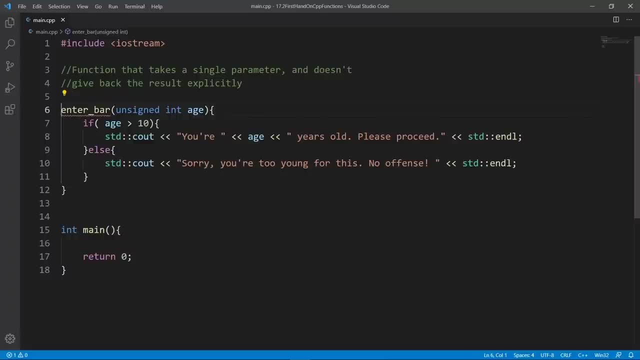 You notice that we have our squiggly lines here. Visual studio code is not happy, So we're going to tell it the return type, We're going to say the function name after that, And after the function name we're going to pass the parameters. 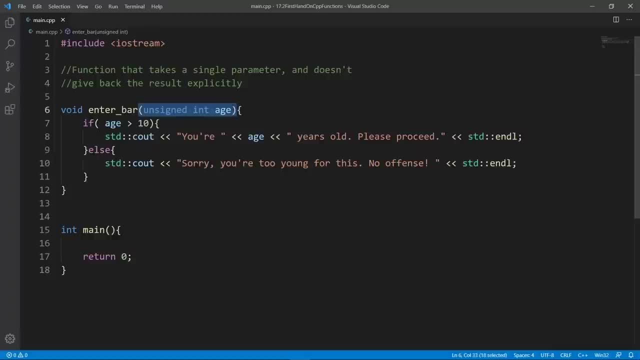 We can have any number of parameters or inputs to the function, but in this case we just have one, because it is enough for our purposes. After that we have the body, and inside the body we do Whatever it is we want to do in this function here, because this function returns void. 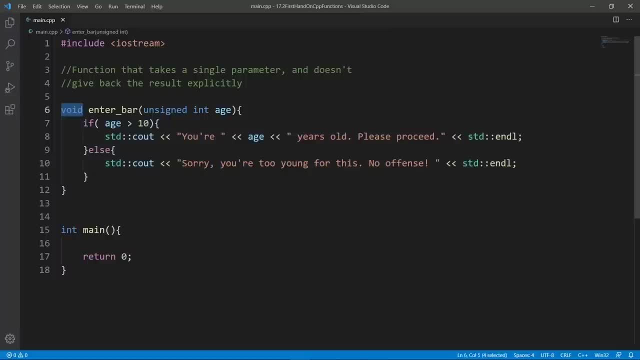 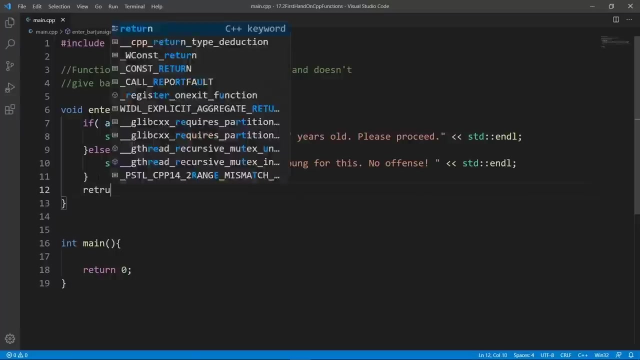 we don't really need to explicitly return from this function here. but this is an exception only for functions that return void. for other return types You will have to put in the return statement. but even for void functions you can put the return statement if you want, and you can do that like this: say return and you're going. 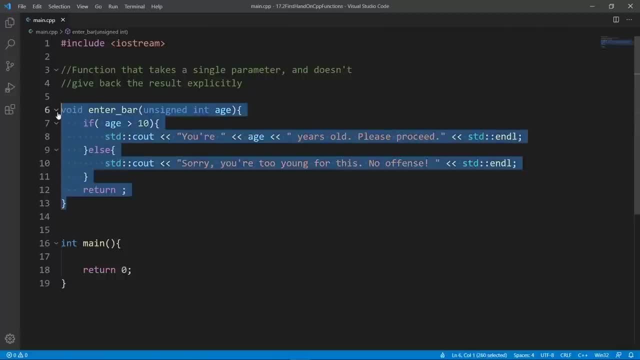 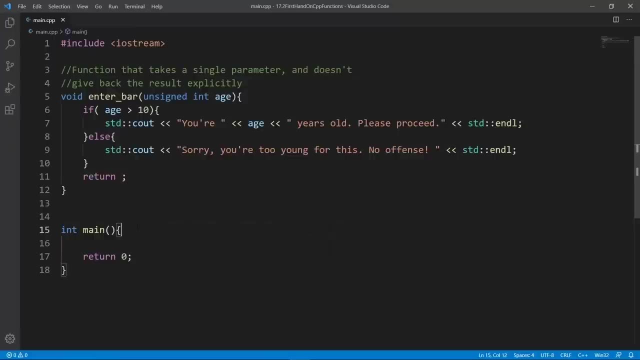 to put a semicolon after this. This is also valid: See plus plus syntax. Okay, Now we have declared that the function it is a valid C plus plus functions. Let's try and call it. We're going to go down in Maine because that's where we want to be calling our functions for now. 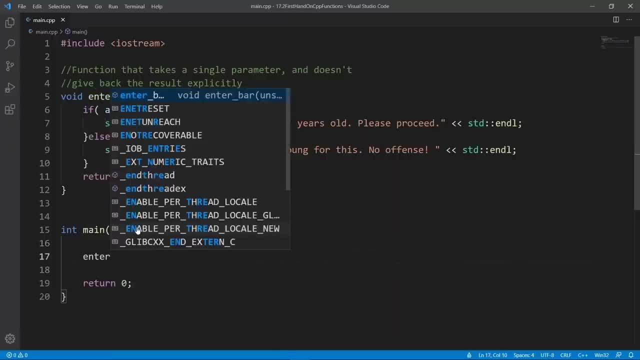 And we are going to say inter bar. We're going to call the function and you use the function name to call it And you're going to put in a pair of parentheses and pass an argument to the function. Again, what you pass to the function when you call it, it's called an argument. but what you pass 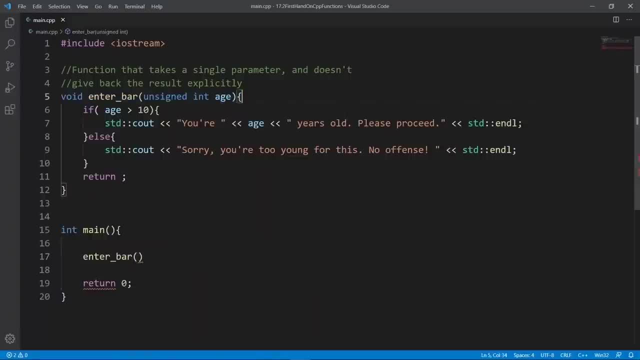 to the function where you are defining it, like we did here. that's a parameter. Okay, So function parameters. when declaring functions and when you are calling the function, what you pass are function arguments, And now we need to pass in some age to this function. 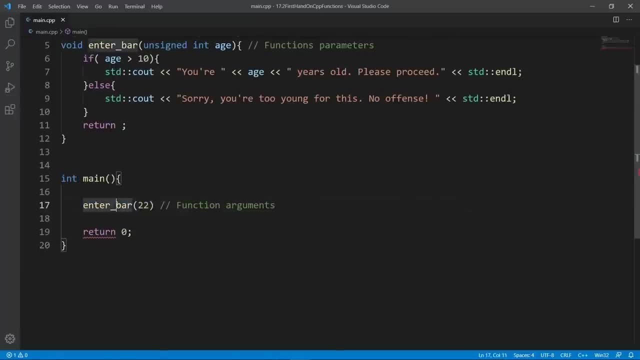 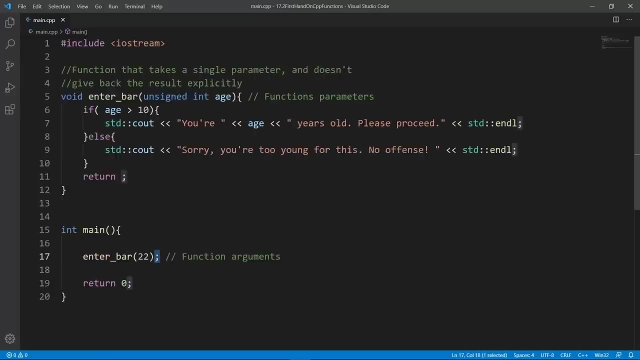 And let's say 22. And if we do that, this is going to be a valid C plus plus program. We've noticed that we have this squiggly line. It is because we forgot a semicolon here, because C plus plus requires to have a semicolon after H statement. 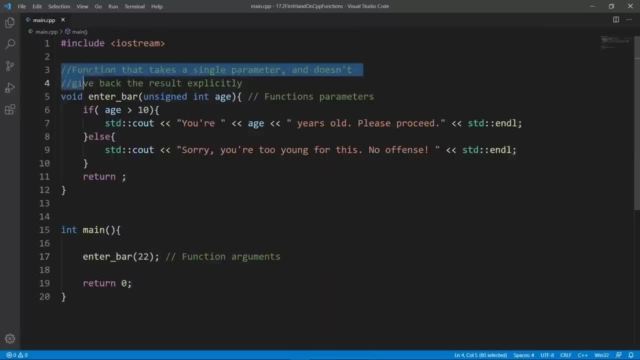 And now we have a valid C plus plus program that is declaring a function and calling a function. down here in Maine We can try to build it. Let's use GCC to do that. The world is going to be good, You see. well, finished successfully, and we can bring up a terminal and actually try to run this. 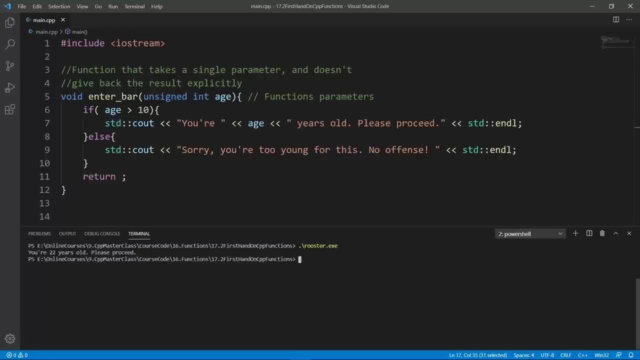 function here. Let's clear and run a roaster, because our program is going to be called rooster, like we have been doing All along, and at the output is going to be: you are 22, please proceed. notice that we have this function defined once, but we can call it multiple times. 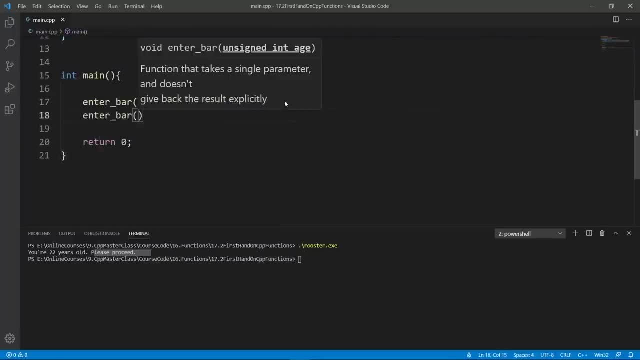 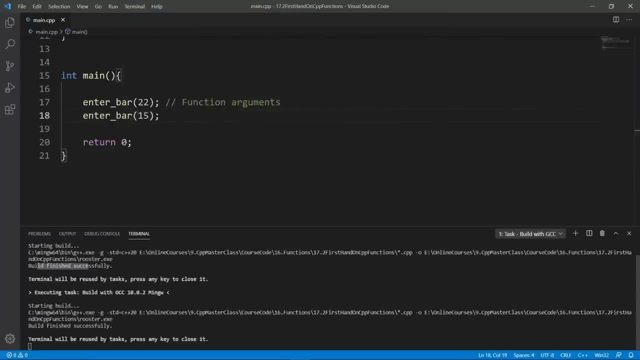 So, for example, if you go down here and say into bar and we give it 15 as the H and we try and build again, let's build with GCC- The board is going to be good, We can clear and run roaster. 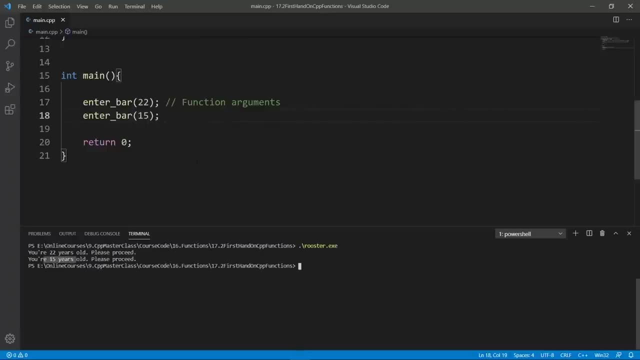 Now it's going to say: you are 15.. Please proceed. Why is that? What are we really doing here? Ah, if age is greater than 10, we say the 10. here we should say 18.. Sorry for this. we're going to build again, and now it should behave accordingly. 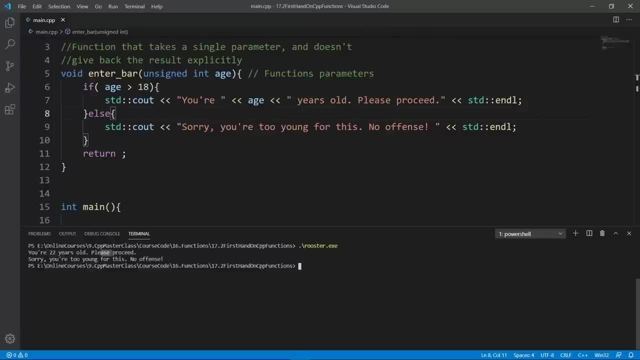 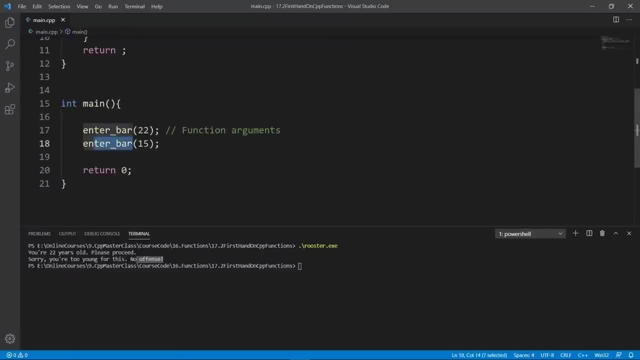 So let's say, roaster, here You are 22.. Please proceed. You are too young for this? No offense, because the age is 15 here. You can keep calling this function and you're going to see things printing out. You can even call this function in the loop. 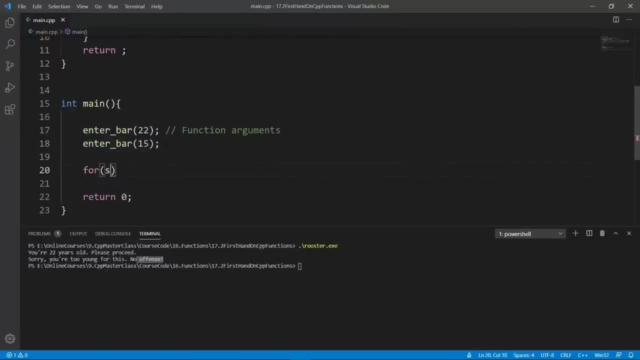 I can't. I can't really resist, So let's do that. We're going to say, for size T, I and say: start from zero, for example, or one, why not? And we are going to say, while I is less than 10 or 20, and we're going to increment. you already know how to use loops. 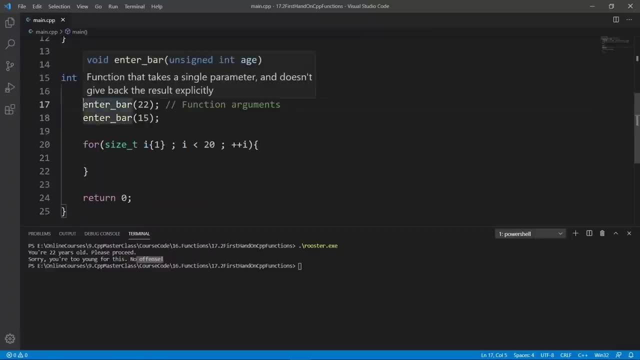 So we're going to be using this as an example and that we can comment out all these guys in front, because we don't want them to print stuff by now, And what we're going to do is call the function with whatever iteration. we are at notice that we have a size T here and the function is going to be taken an unsigned integer. 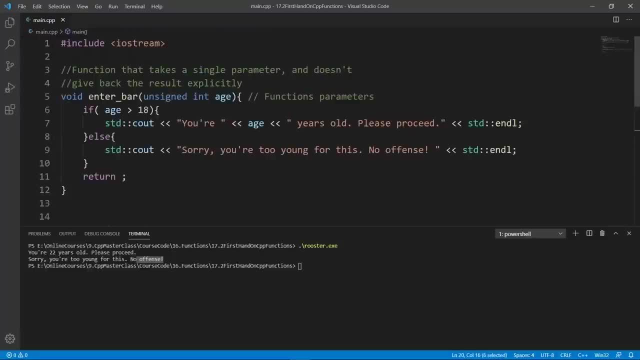 So we're going to have implicit conversions from size T to end, or, if we really want this to not cause any problems, we can change the type of our parameter to be size T. This is also valid C++ code. Let's say size T. 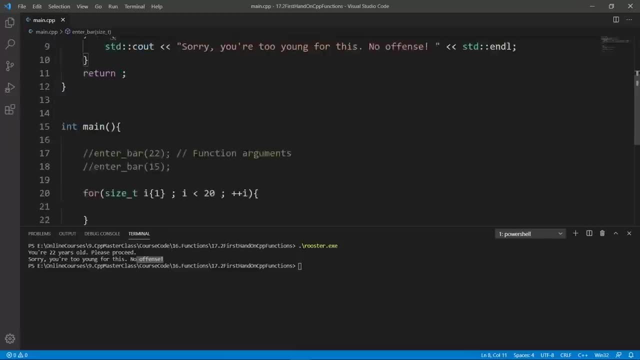 T properly, And if we go down here we're going to say enter war and we're going to pass an eye. Watch what is going to happen. This is going to loop from one all the way to 19 and it's going to be called in this function with whatever iteration we might be at. 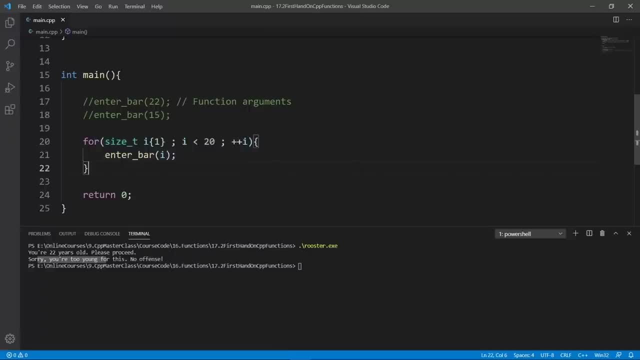 So it's going to look from one all the way to 18 and it's going to tell us we are too young for this, but for 19 it's going to let us in because we will be Old enough to enter a bar. 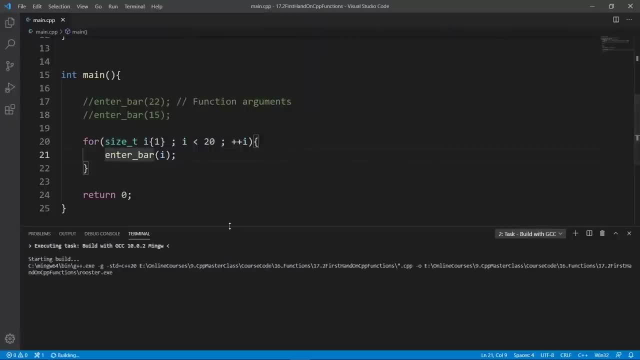 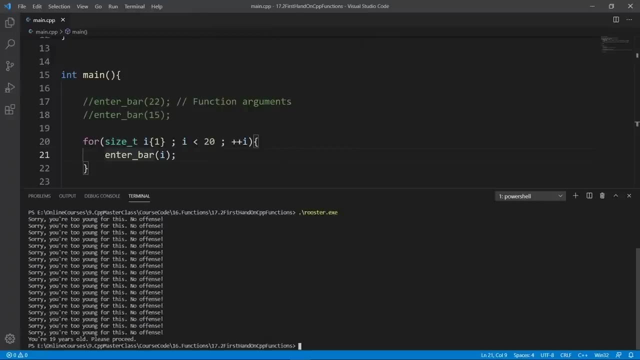 Let's try this. I think it's going to be fun. We're going to world with GCC and we're going to clear and run rooster- Ah sorry, You're too young for this, You too young for this- And once we hit 19, it's going to tell us we are young enough to enter a bar and we're going to go in and have as much fun as we want. 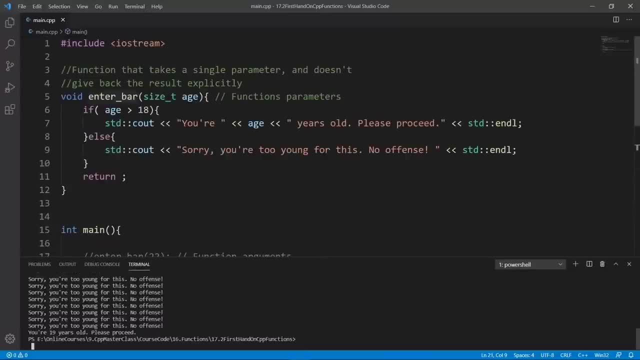 So this is really how you can declare a function. Remember, a function is uniquely identified by its signature, And the signature is really the name of the function and the parameters that you have in here. Okay, Once you have the function declared, you're going to do whatever you want in the body. 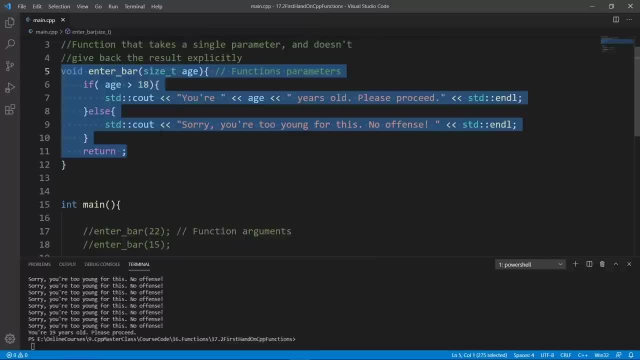 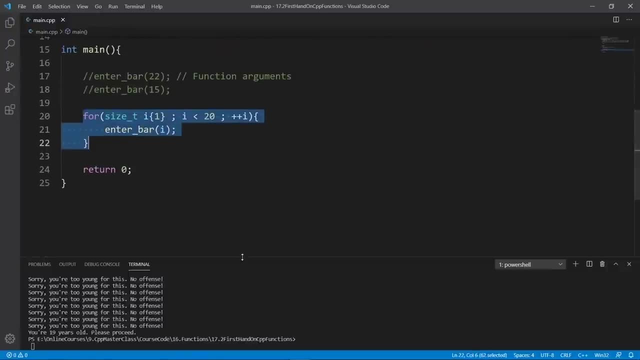 You are going to optionally return something from the function And once the function is declared or set up, you can go in main and call it and do whatever it is you want with it. Okay, Now I think we are mature enough to try out a few other functions. 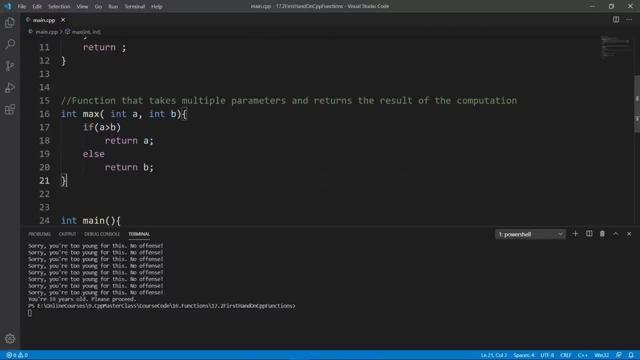 Let's go down and put in another function which is going to compute the maximum of two numbers. The signature of this function is going to be its name here and the parameters. Notice that we are taking two parameters because we want to be computing the maximum between two numbers. 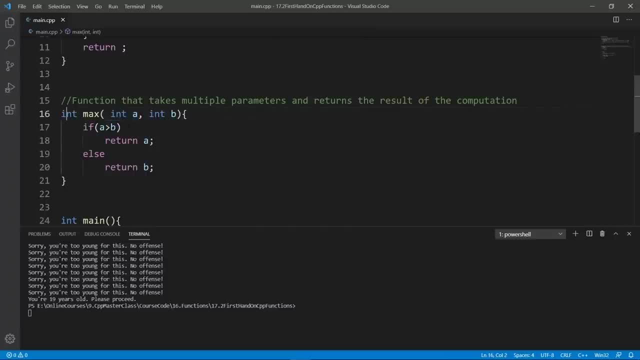 And this function is going to return something. We want to get the maximum out of the function and use it to do something else when we call it. So this is the declaration of the function. Once we hit the body of the function, we are going to compute the maximum. 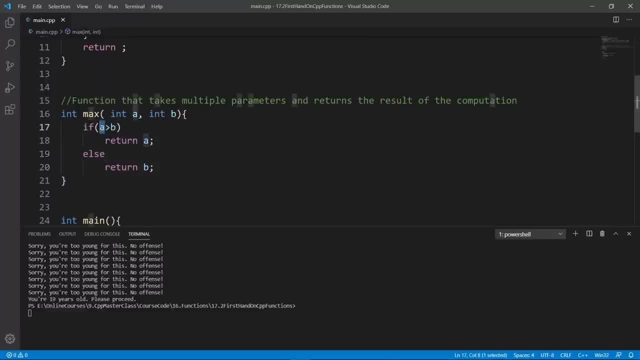 We're going to say if A is greater than B, then A must be our maximum. So we're going to return Turn that. And if A is not greater than B, then B must be the maximum. We're going to return B as our maximum here. 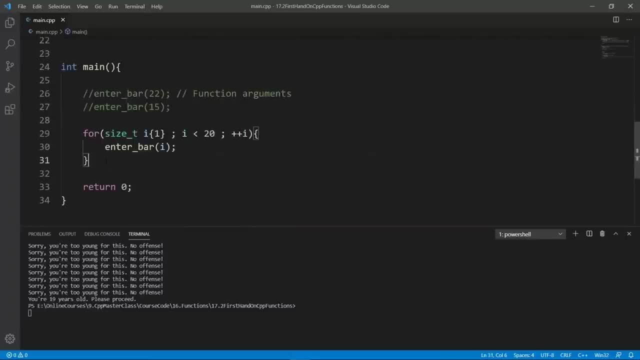 This is what the function is doing. We can go in main and call it. Let's go down and comment this out, because we don't want noise output from these guys, So call it interbar. That's what we were doing. Now we are calling max. 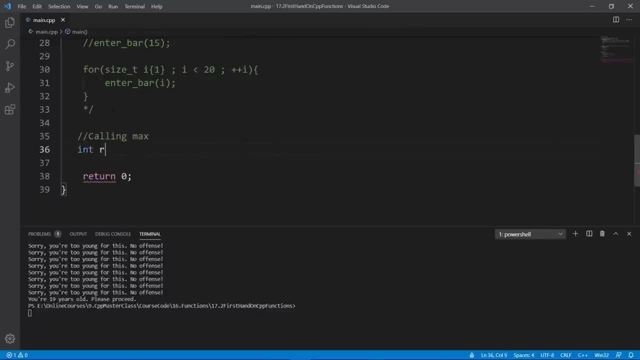 So we're going to go down and set up a variable Call it result- Why not? And we're going to compute the maximum between 10. 20. Why not? Okay, So let's see what we get, And we're going to print the maximum this time. 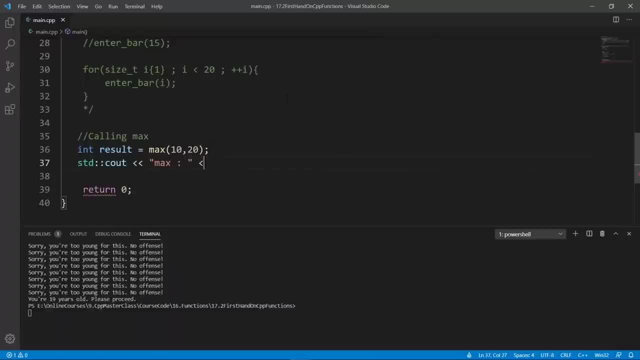 We're going to say: max is result. Okay, Now, if we build this program and run it, try to guess what we're going to get. We're going to call the maximum function And what we pass in here are arguments. Again, we are not passing parameters here. 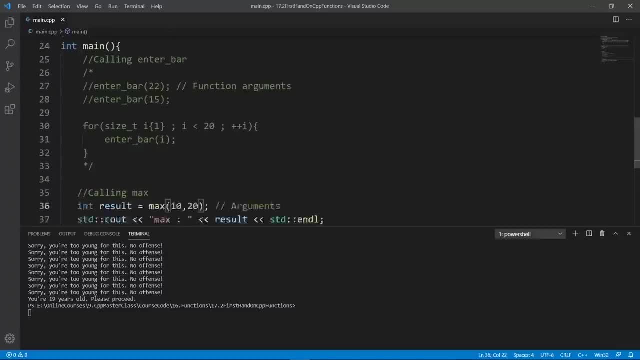 We are going to pass in 10 and 20 as our arguments And when we call the function, control is going to jump to the body of the function And we are going to fall inside here. The arguments we're going to pass in are just going to be copied in the function. 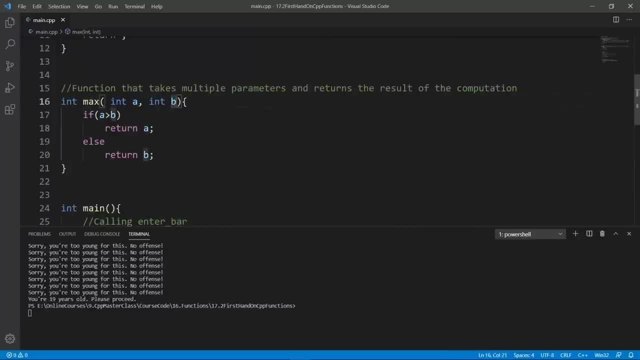 And we will have them through these names, A and B. So we're going to test and see if the first parameter is greater than the second. In this case, the first parameter is not greater than the second because the first one is 10.. 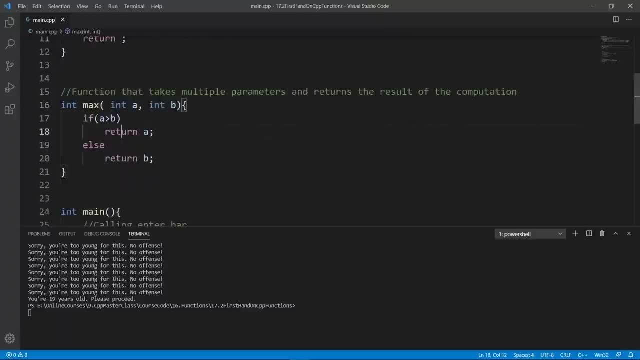 The second is a 20. Let's go down and see that And the test here is going to fail And we're going to run whatever is in the else block here And we are going to return B as Our maximum. When we return B, B is going to basically be the result of this expression here. 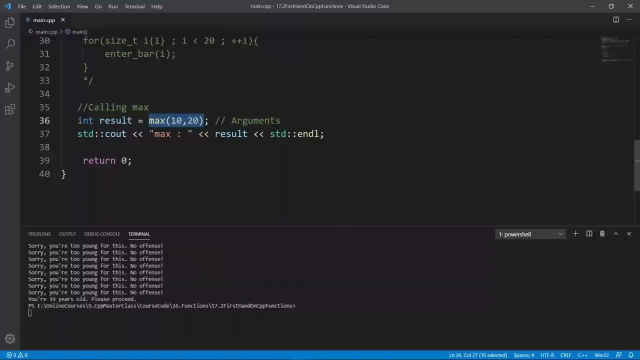 And that result is going to be assigned to our result variable And we're going to print it out with this stdcout statement here. So let's try and build this. We're going to build with gcc. Again, the build is going to be good. 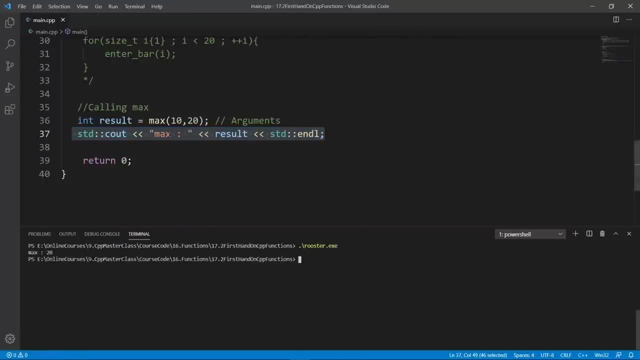 We're going to clear and run rooster. You see that maximum is 20.. If we try and change this- for example, make the first parameter 100 and build again, Let's see what maximum we get. I'm going to clear and run rooster. 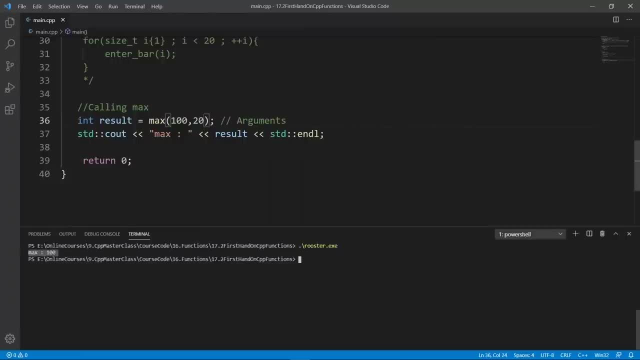 I'm going to say that maximum is 100.. And again, you can call this function however many times you want. For example, we can call it again and say: reserved equals max, Using two variables that we have, Let's say x and y. 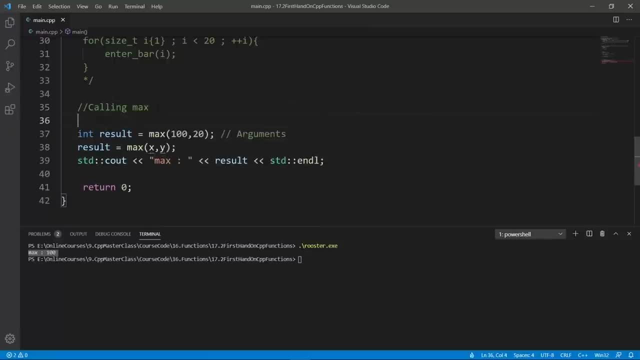 And go on top and declare these two variables. Why not? We're going to say int x And we're going to put in a 22. And we're going to say int y, Y and put in a 44. Why not? 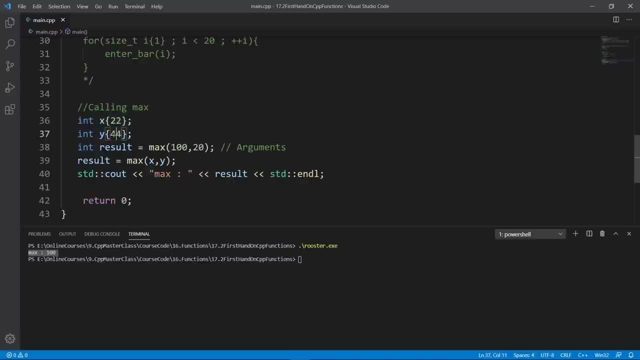 And now if we print the result, we're going to get 44.. Because that's the maximum that was assigned back to our result variable. here Let's build again. We're going to run the task to build with gcc. You can clear and run rooster. 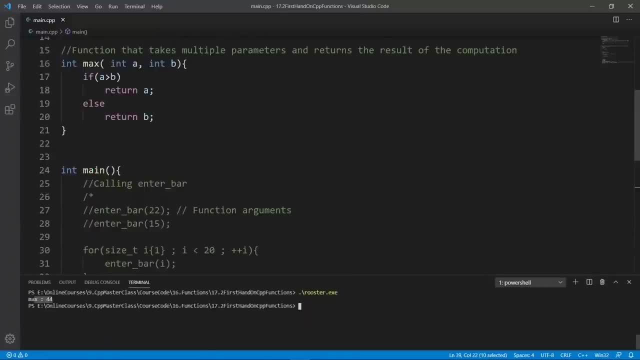 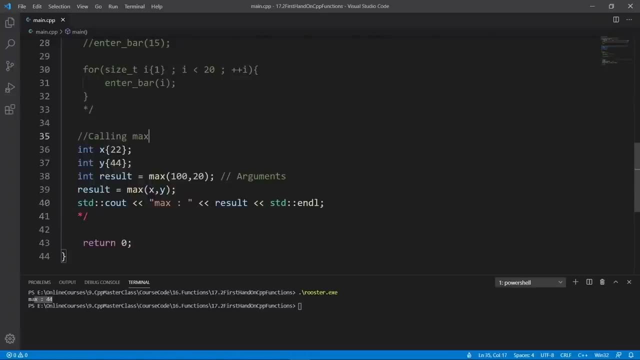 You see, max is 44. And this is really how you can declare and use a maximum function like this. We're going to comment this out Because we have a few more Functions we want to try out. Let's go on top and put in another function. 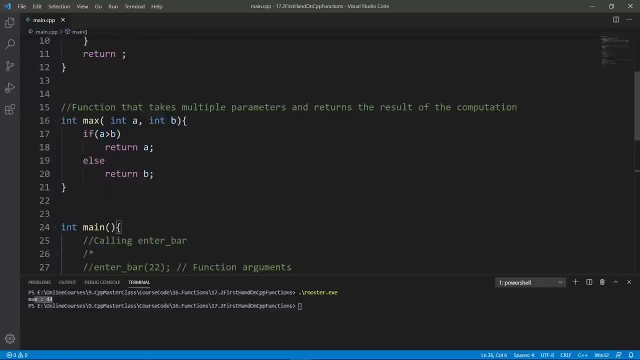 And again notice that we are declaring functions before the main function here. This is a requirement of a C++ compiler, Because before you use the function the function must be declared somewhere. So we need to go before the main function and declare our functions here. 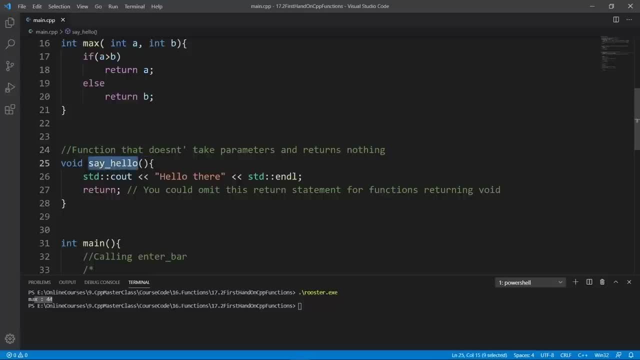 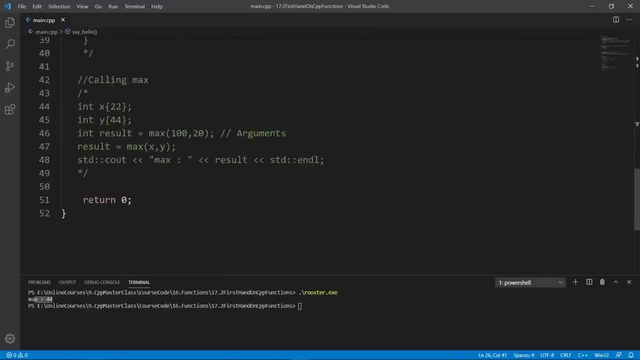 The function we're going to do now is say hello here. It's not going to take any input And it's not going to give us any Output. It's just going to say hello and die off. We can go down and call it. 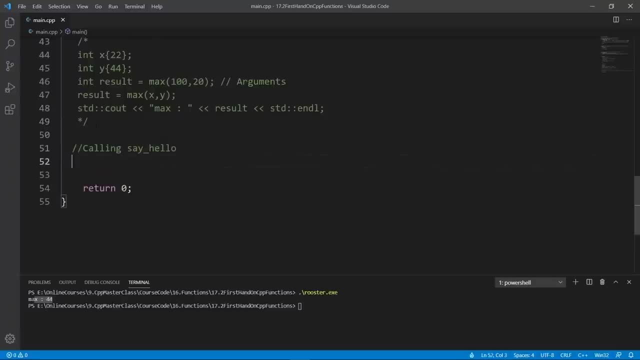 This is going to be super easy: Calling hello, And we're going to call it. Say hello. See that even Visual Studio Code knows about this function. We can call it like this: It's going to be activated, So we're going to hit the body of the function. 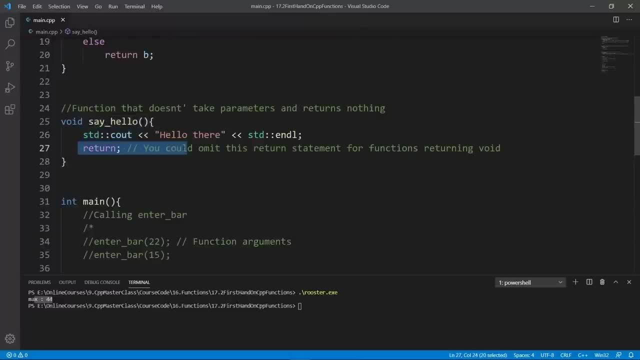 We're going to say hello there And the function is going to return or die off. Please know that you could omit this return statement for functions that return void. So if we comment this guy out, The function is going to work equally well. 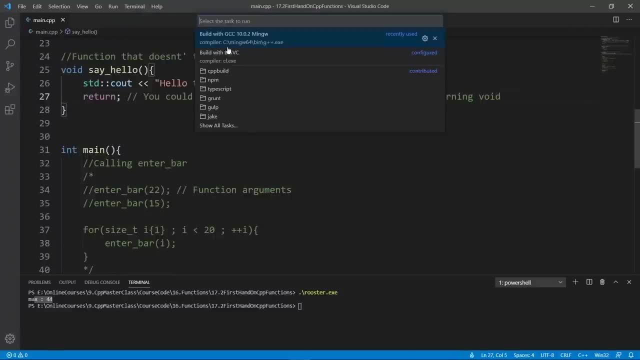 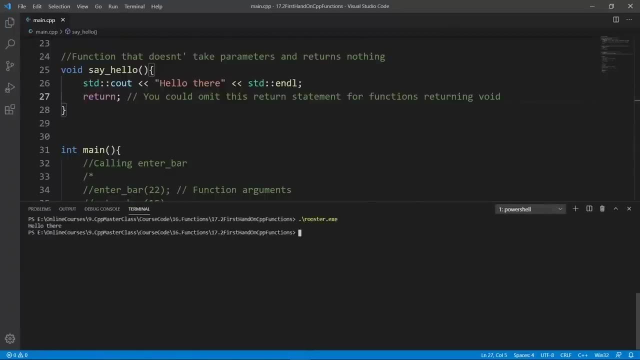 You can use this however you want. Now we're just going to build with GCC and see this function run. The build is good. We're going to run rooster And it is saying hello there. Let's go down and look at another example here. 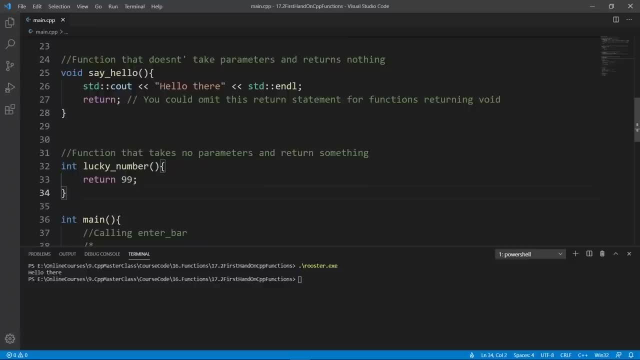 The next function is going to be lucky number. It's not going to take any input, But it is going to give us an output in the form of an integer, So we can call it. Let's go down and comment out Saying hello here. 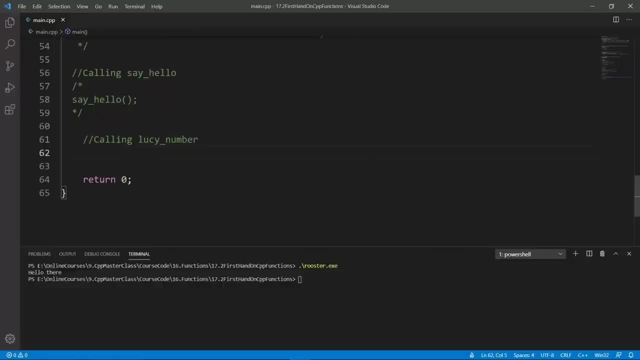 And say that we want to call lucky number And we can go down and set up a variable. Let's do that. We're going to say int result And we are going to brace initialize this guy. So it's going to be initialized to zero. 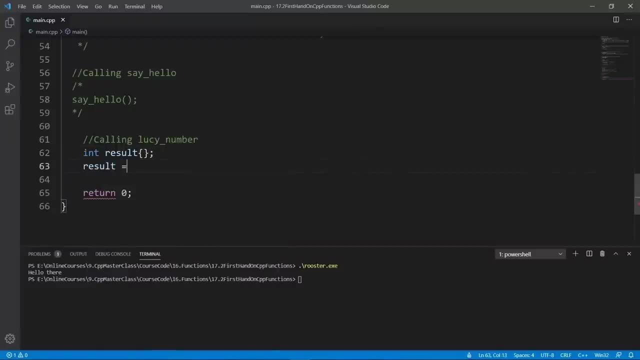 And we're going to say: result equals lucky number And we're going to take the result returned by our lucky number function And assign that to the result variable And we can print it out if we want. So we can say stdc out and say result and we're going to put that out here: say result. 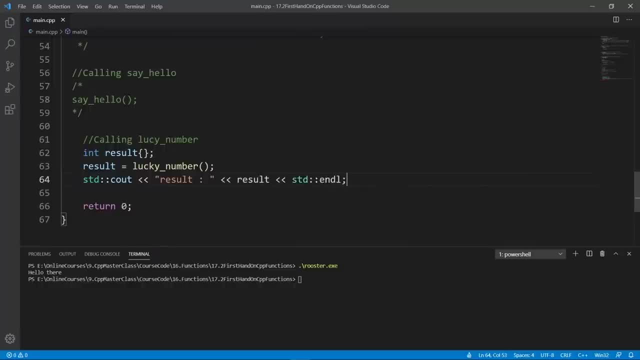 and if we build and run this program, we're going to get this guy printed out. We should see a 99, because that's what we are returning from our function here, and result is 99, as you see in the output here. So this is really how you can declare your functions. A function has a unique. 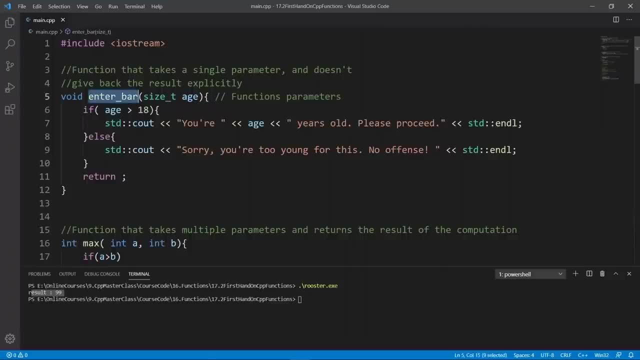 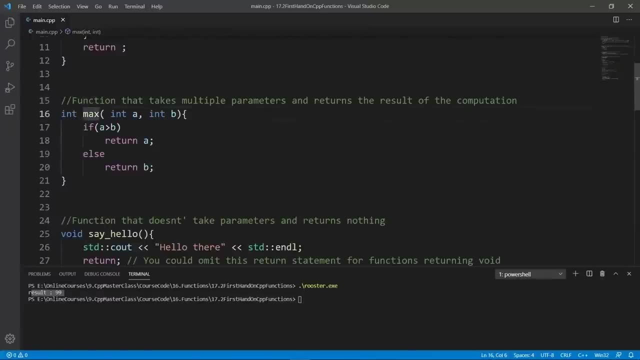 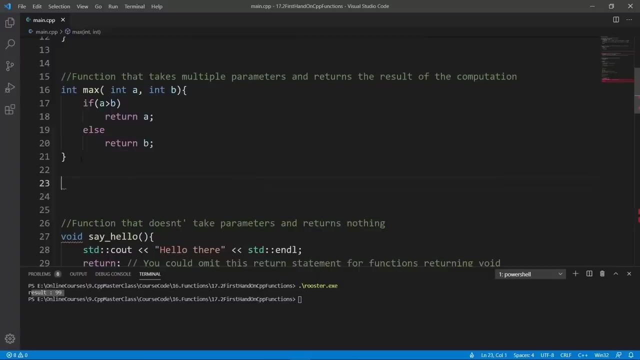 signature. so, for example, intobar here has this particular name and these parameters. here, If you go down, max has its own name and the parameters that it takes in If you go down, say hello and lucky number, are different in their own ways. If you try and set up another function. 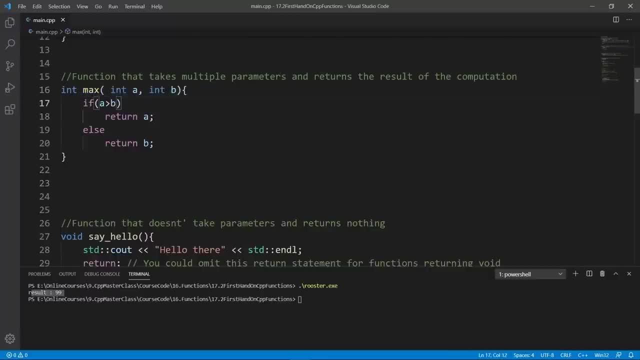 that has the same signature as max. here your compiler is going to be able to say hello and it's going to freak out. Let's try and do that. We're going to set up another function. It's going to have a void return type. We're going to call it max because we want to match this signature here. 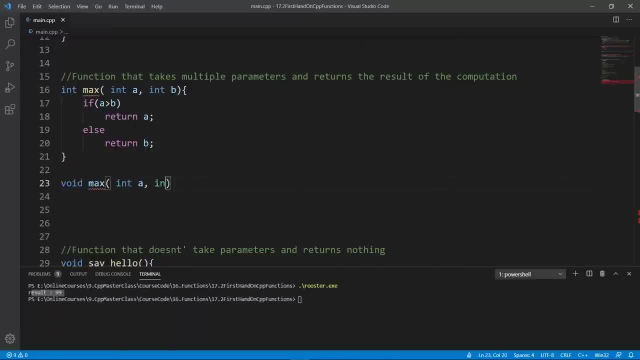 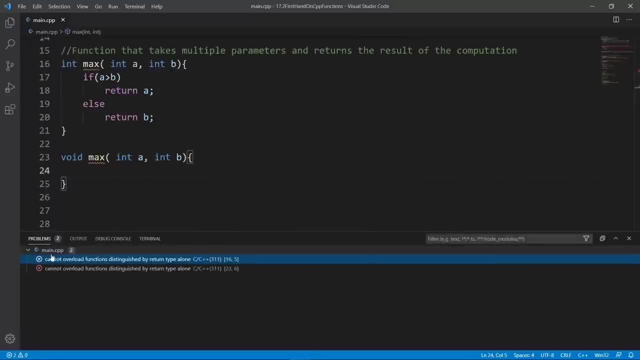 and we're going to give it two parameters, int a and int b, and we can do whatever we want in this function. Notice that we have a squiggly line. If we open our problems tab here, you're going to see that Visual Studio Code has a few problems with this because we are setting up a function with 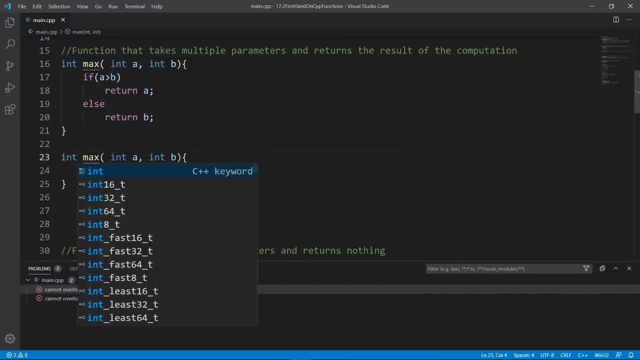 the same signature twice. Let's try and even make this a net and see what we get. Right now we don't seem to have a problem, but if we get to run this program we're going to have problems. Let's go down and actually activate. 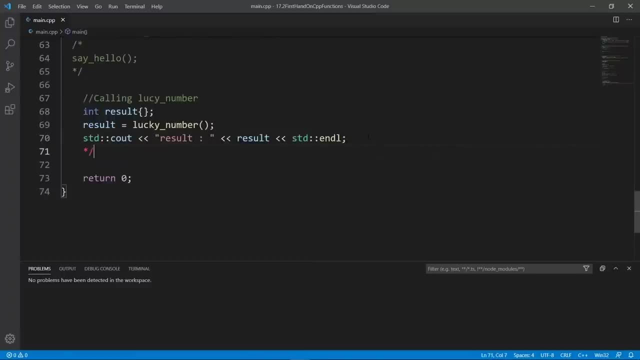 the code to call the max function to really show you this, because you need to know. So we're going to comment out calling lucky number and we want to call max, We're going to activate the code to call max and we are going to world this with gcc. Notice what we're going to see. 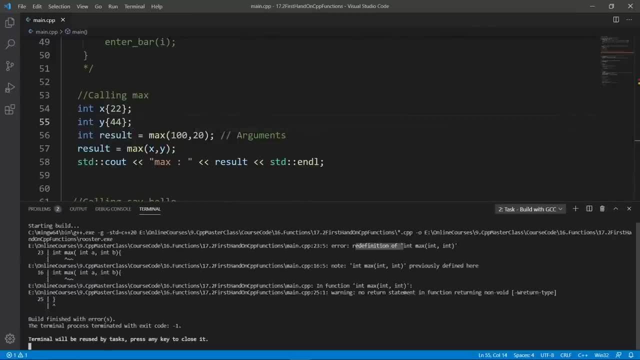 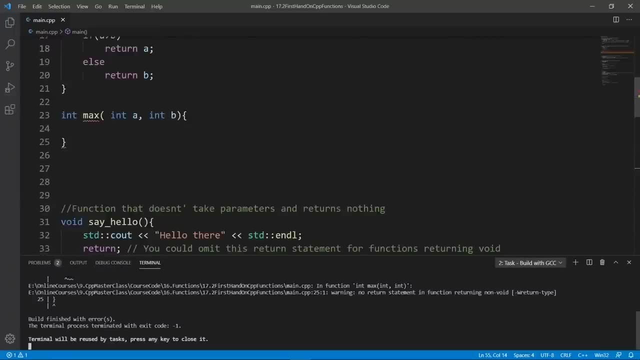 We have problems here. We have a compiler error saying redefinition of int, max, int, int. and one might think: what if I name my parameters differently? here, For example, I call this guy c and this other guy d. Let's do that. Using different names like this is not going to solve your troubles, because 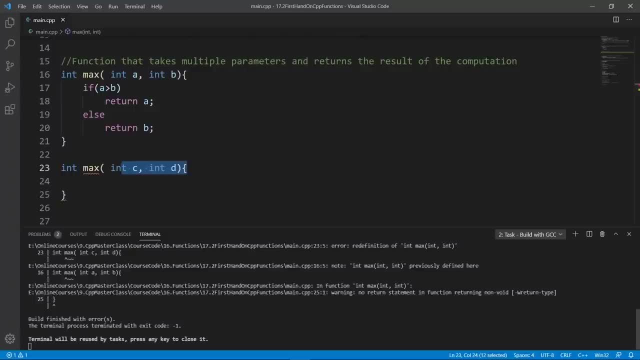 if we try and build again, we're going to get the same compiler error. This is not going to change your thing. We don't have enough tools to really understand this problem, but know that you can't have two functions with the exact same signature in a single C++ program, and we're going to learn more. 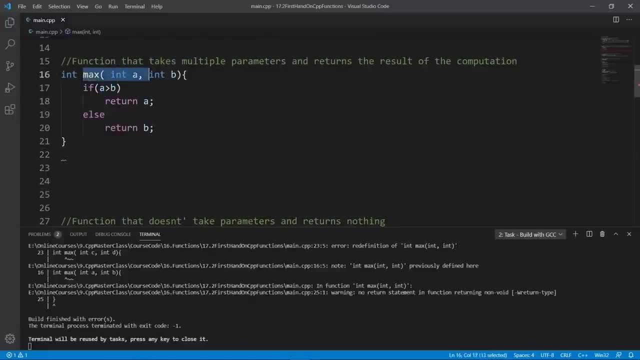 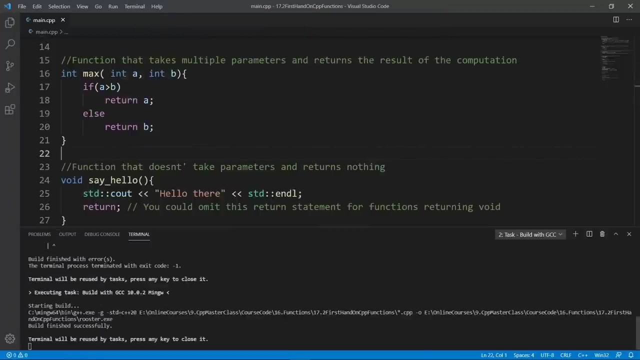 about this later, but know that the signature of a function must be unique to it throughout your entire C++ program. If you remember this simple rule, you're not going to have many problems. So let's try and build again to make sure we have no more problems in here. 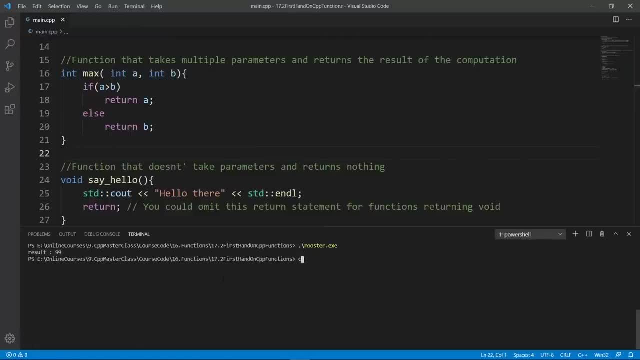 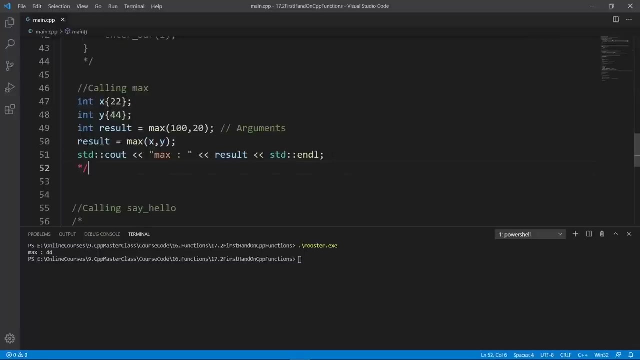 The build is good and we can run the program to see our maximum printed out. So let's do that clear. rooster and max is 44. It is exactly what we expect. The last thing I want to do in this lecture is make it super clear in your mind that what we pass to functions we have been setting up. 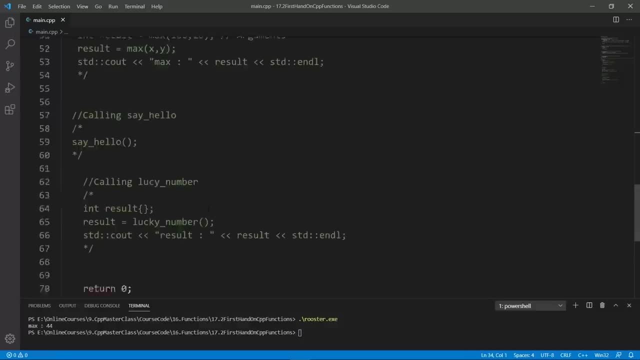 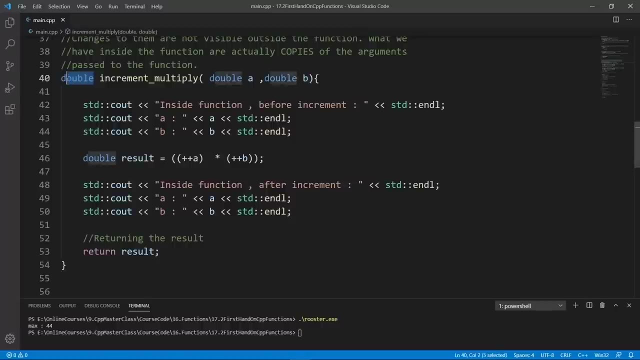 so far are copies. So let's go on top and set up a simple function. The function is going to increment and multiply. It returns a double type. The name of the function is increment and multiply and it is going to take two parameters in: A double a and a double b. Once we hit the 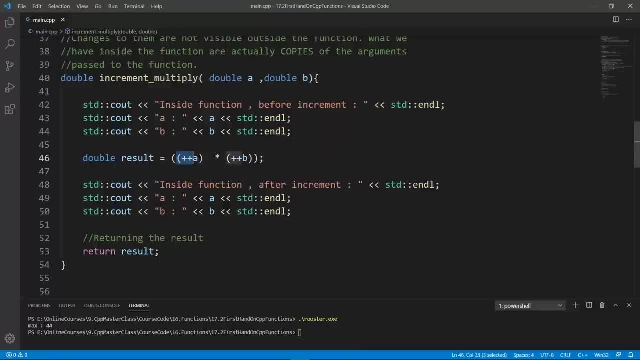 body of the function. we're going to increment a and b, The arguments that were passed to the function, and we're going to multiply them and we're going to store the result of that in a result variable. The result variable is what we're going to return to the function and whoever called 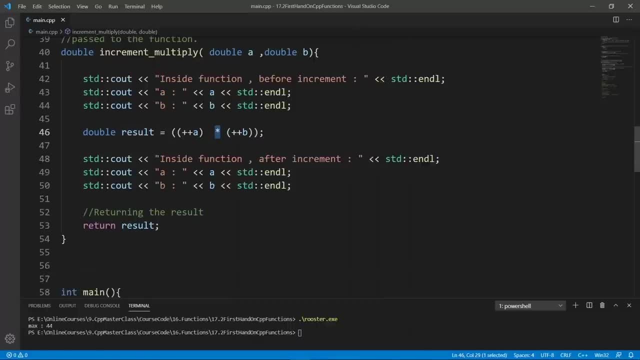 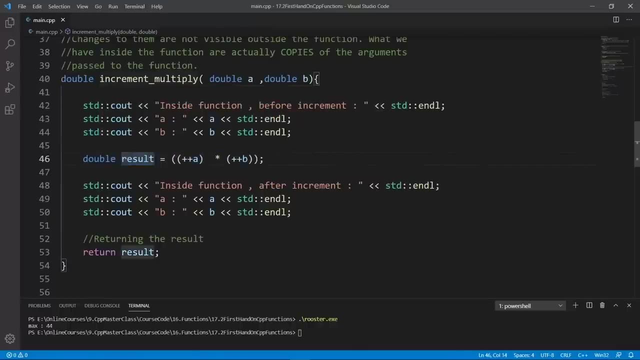 this function is going to use it in the next lecture, So let's go ahead and do that, To do whatever they want. What we really want to see is that the changes we do inside the function are not going to be visible to the arguments that we pass to this function here. To really make this: 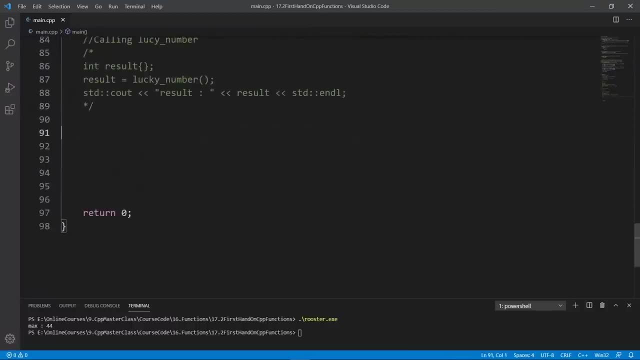 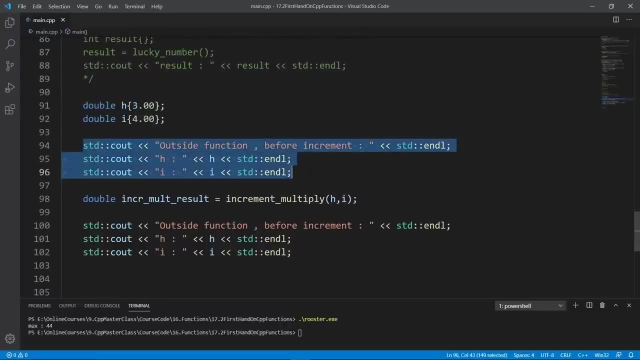 super clear. let's go down in main and set up a few variables. We're going to have a double h and a double i. The values are going to be three and four. We're going to print them out and we're going to call our increment multiply function. Notice that we pass h and i and we're going to 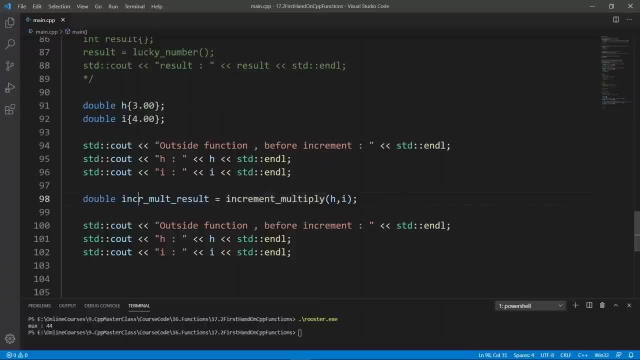 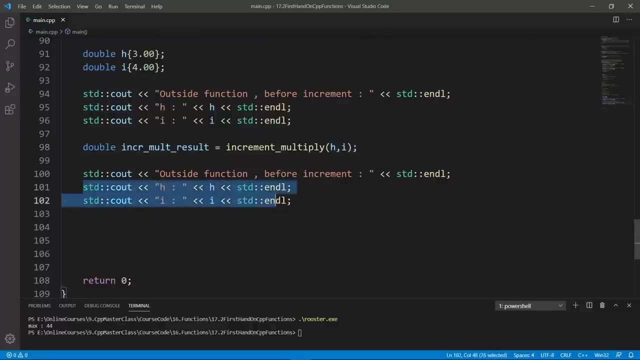 increment multiply to the function and the result of the function is going to be stored in the increment result variable here. But the return value is really not important. What we want to see is if the changes we do to the arguments are going to be visible on the outside of the 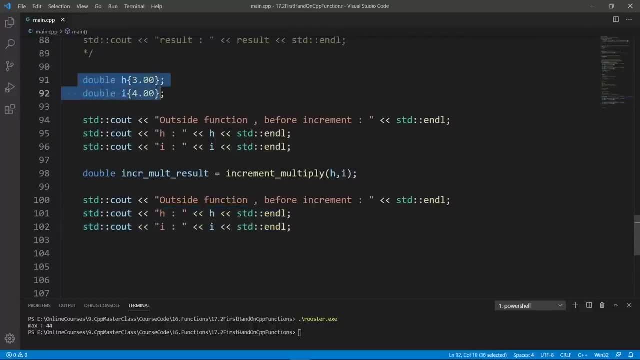 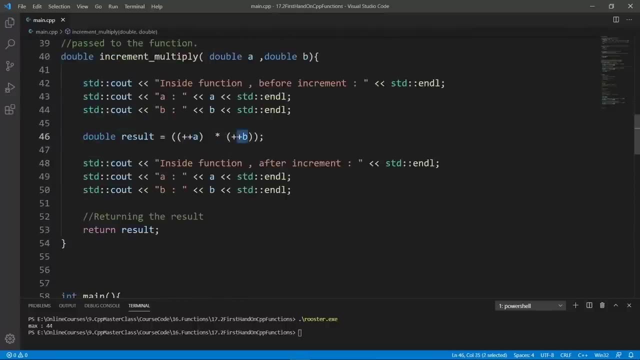 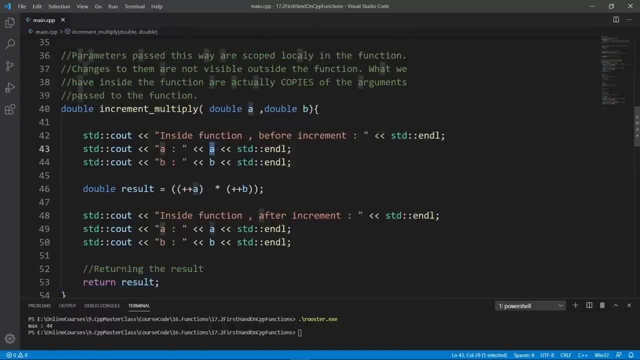 function here. So remember, we have h and i here. We pass them to the function. Once we hit the inside of the function we're going to increment a and b and we are going to return from the function. So let's see if a, which was a three, and b, which was a four, have been incremented to. 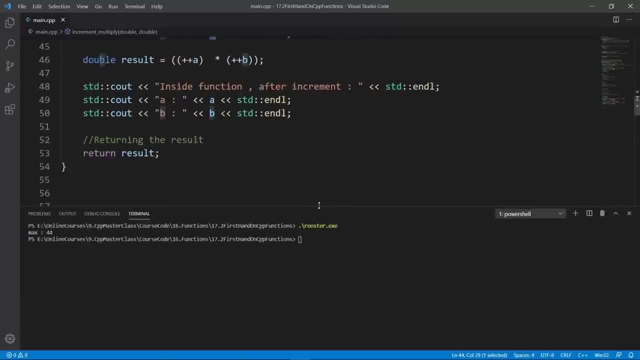 four and five. That's what we want to see. So we're going to build this and run this. So let's use gcc to do that. The build is going to be good. We're going to clear and run, rooster and notice. 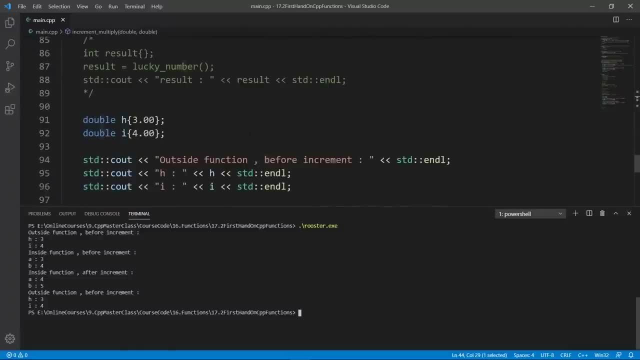 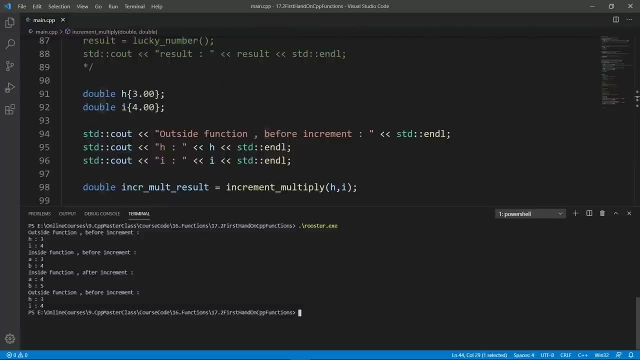 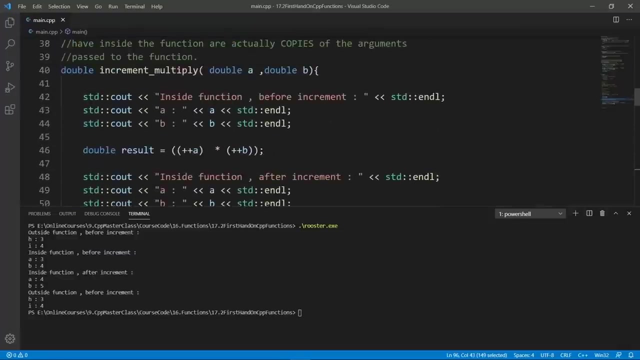 what we have here. Let's go down and look at the variables again. We set up h to contain a three. We increment h and i are four. Okay, so that's what we're going to print here Once we hit the inside of the function. we are going to say what we have inside the function before we do the 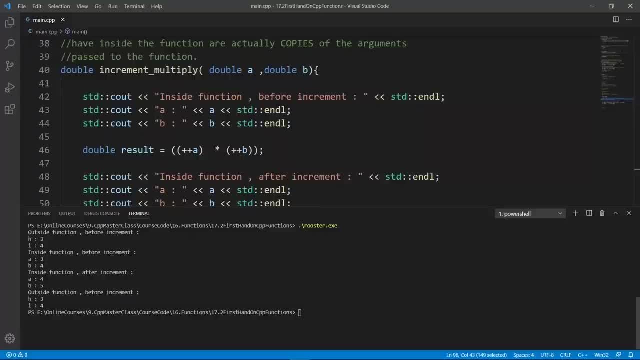 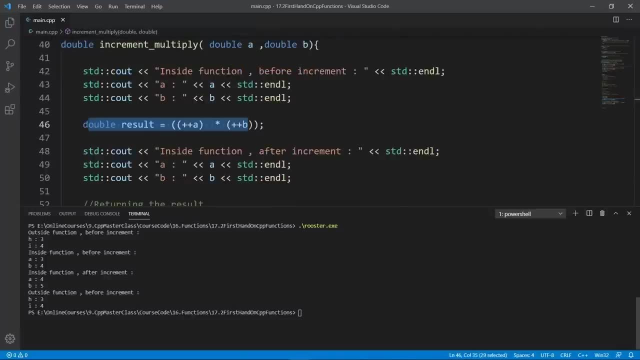 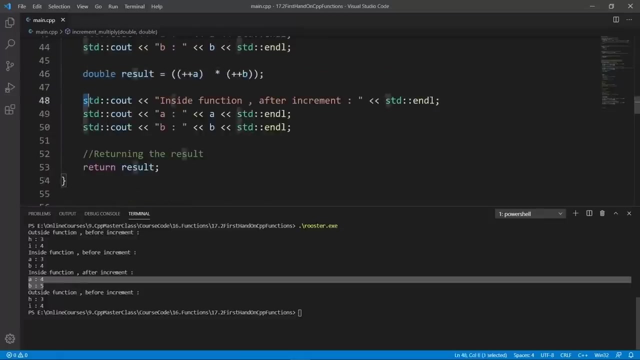 operation. before the increment: Again, a and b are four. So these are copies we have inside. We're going to do the increment and after we have the increment, a and b are going to be four. But once we're done with this guy here, we're going to see that h and i are still three and four. So we didn't. 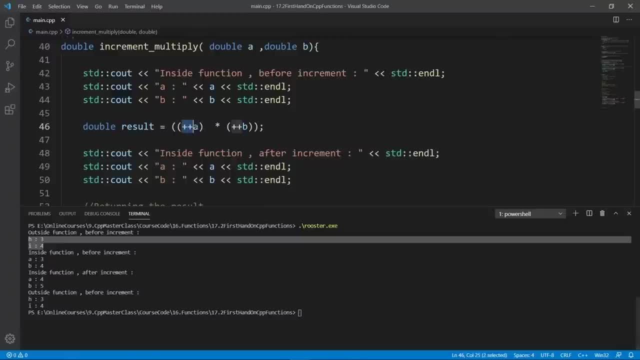 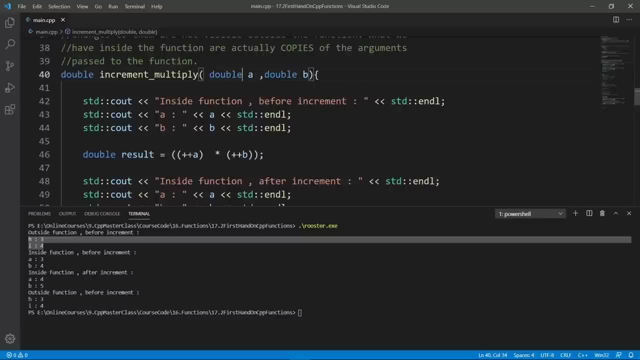 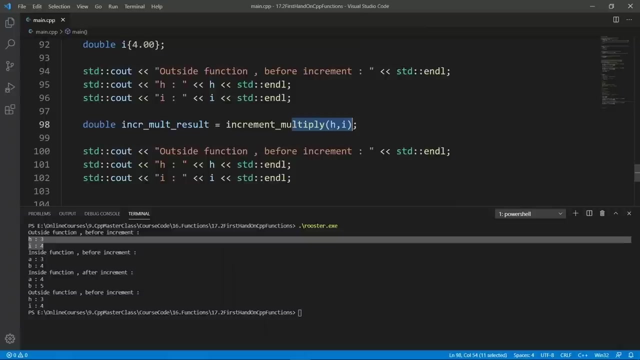 really affect h and i. when we did this increment here. What we affected are copies that were passed to a and b here, And this is something you need to know because some people will think that because a pass h and i in my argument list here, I can manipulate h and i. What you are manipulating. 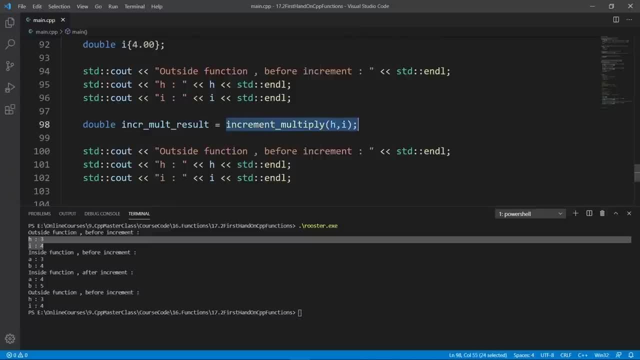 is that we're made by the compiler to pass the arguments to the function here. This is something you need to keep in mind and we will learn more about this, But I wanted you to learn this firsthand, And this is really all we set out to do in this lecture. I hope you have a better. 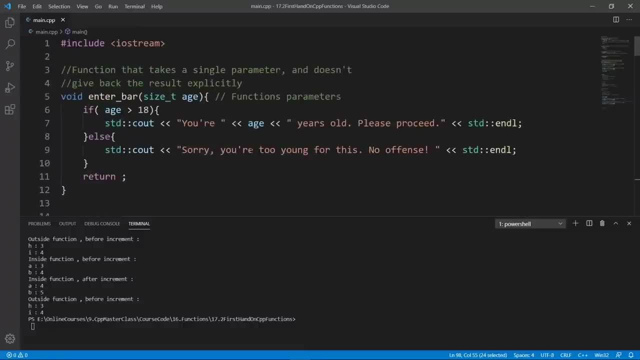 understanding of what a function is and what you can do with it in C++. We are going to stop here in this lecture. In the next one we're going to learn a little more about function declarations and function definitions. Go ahead and finish up. 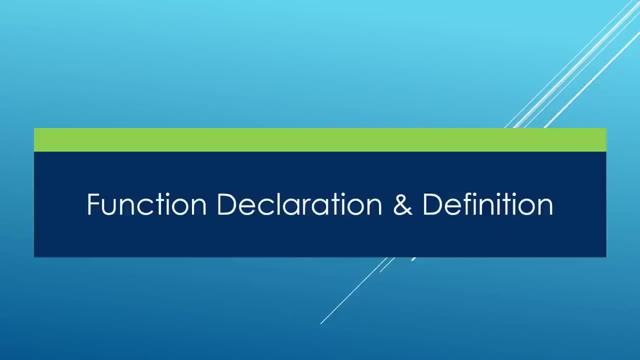 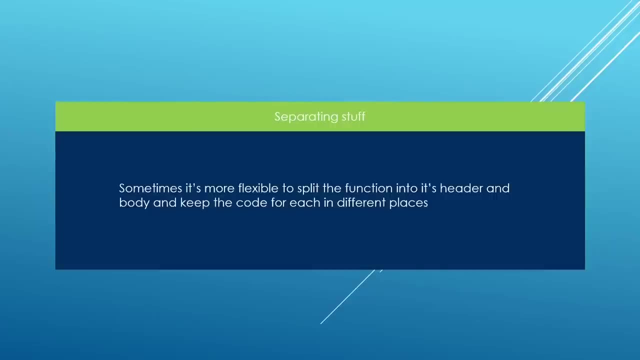 here and meet me there. In this lecture, we're going to learn about function declarations and function definitions. The motivation for the topic we're going to be talking about here is that sometimes you really want to separate a function header from its implementation because you don't want to expose all the details about how you do stuff. Let's look at a simple example. 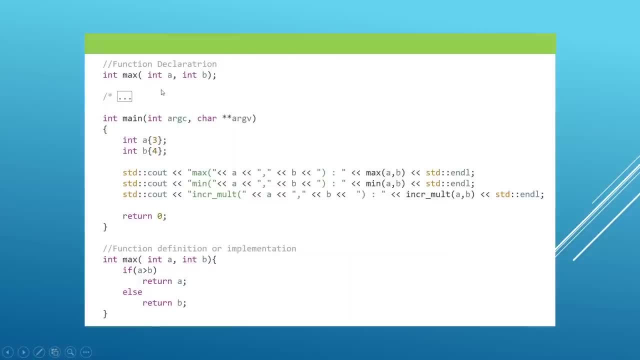 In the last lecture we declared a max function, which was computing the maximum between two functions. The output was an integer, so that's what we returned. The name of the function was max and we had two parameters, int a and int b. But what we did in the last lecture was cramp the 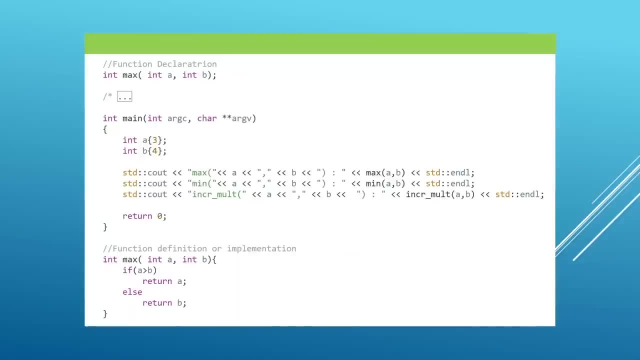 entire function body in front of main. but sometimes people don't want to really see the details of how you do stuff. They just want to know a summary of what your function does, what we can get out of the function and what we need to give to the function for it to do its job. 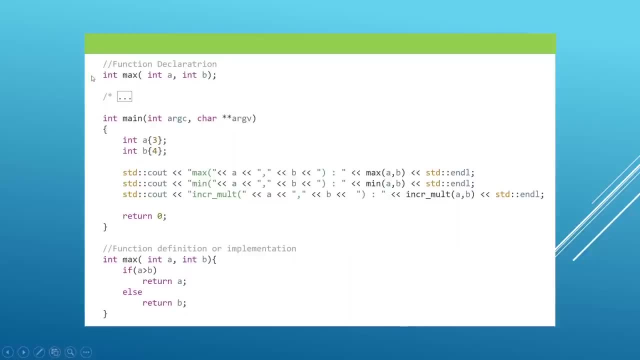 And that's what we're going to do next. If you look here, we have the function header in front of the main function, and the function header is made up of its return type, the name of the function and the list of the parameters, and after that we're going to put a semicolon. This is called a function header or a prototype. 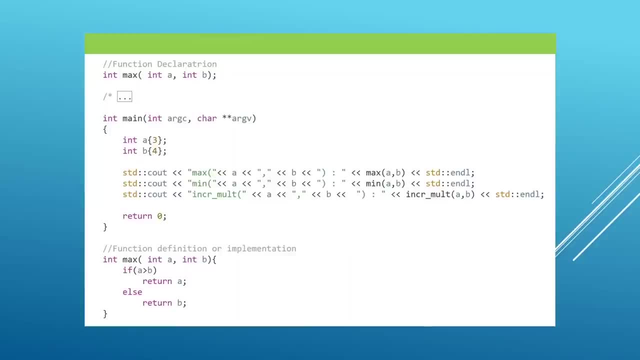 and when we do that, the compiler is going to be happy and it's going to work with us to compile our program. but when we get to link our program to really put it together and make one binary, the definition of the function is going to be needed. And if you look after main here what we 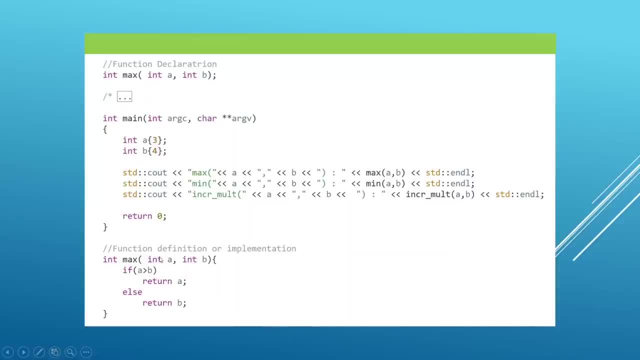 have is our function definition. If you look closely, you see that it is exactly the same thing we had in the last lecture. We have our header information, We don't have a semicolon after our parameter list, but we have a pair of curly braces and inside these curly braces we have 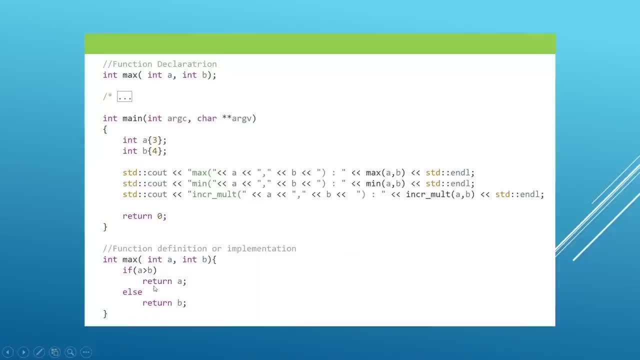 the body of our function. Now it is really easy to look at this function and see how it works. So we're going to look at this program because we don't have to look at all these details about how this function works. We can get first-hand information on how we can use this function. 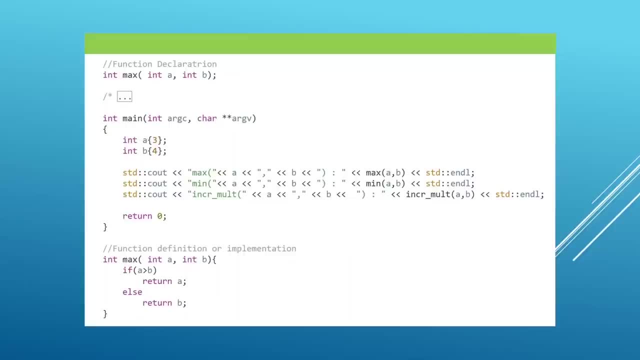 and that is what most people are going to be interested in about your function. They won't really want to go in and see how you do stuff. they will want to use your function to get the output and use it to do whatever it is they want to do. If you look here in the body, 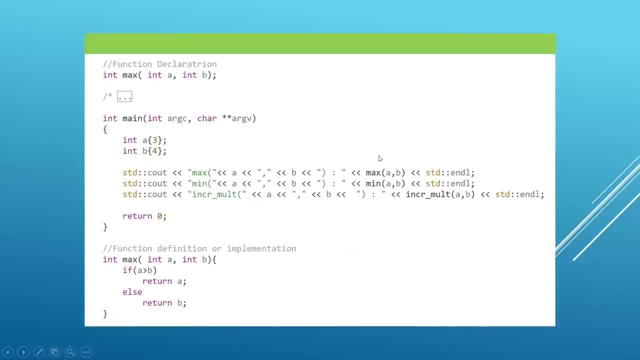 of the main function. we have two variables, a and b, and we use them to call the maximum function function. We can also set up a minimum function which works in the similar way and we call another function called increment, which is going to increment and multiply. whatever arguments we 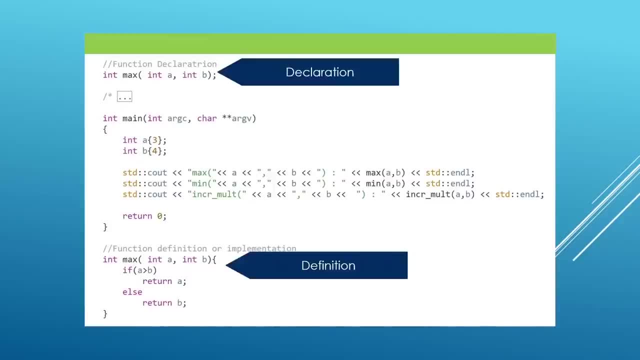 pass to this function. So the main idea here is that we can split our function in two parts. One is going to be the function header, which is really going to be the function declaration, and the other is going to be the function body with all the details about how the function works. 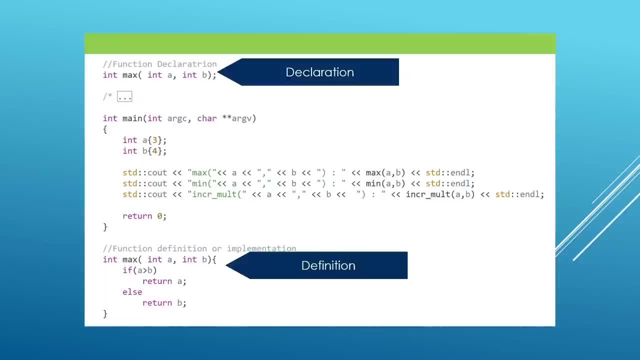 and that's going to be our function definition, And once we have these two things in place, we can call the function in our main function and do whatever we want with it. Okay, now it should be super clear that we can separate our function in two parts- declaration and definition- and sometimes 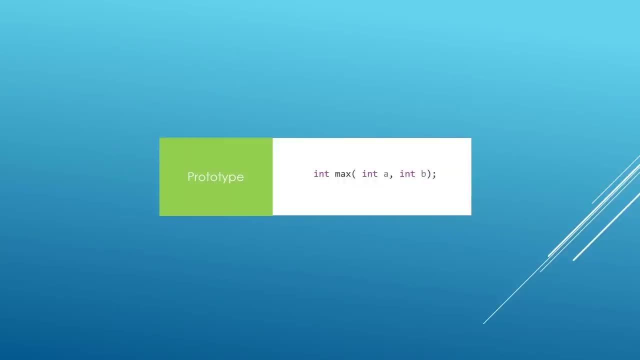 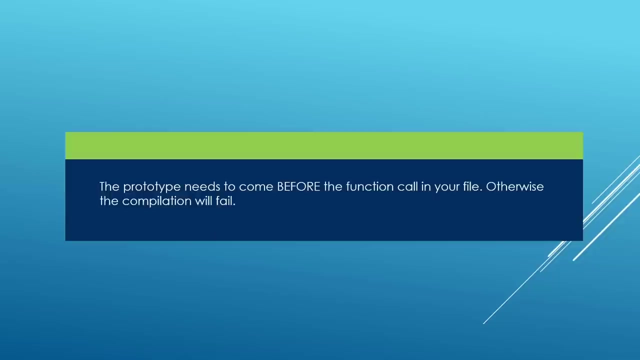 the declaration part is also called a prototype. That's a prototype of a function and it is made up of the return type, together with the function name, together with the parameters, and after that you're going to add a semicolon to make it valid C++ syntax. And another thing you should know is that the prototype needs to come before 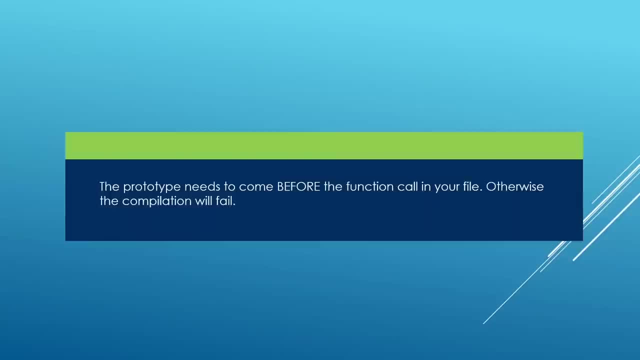 wherever it is called. If you're trying to call a function before its prototype is seen in your C++ program, you're going to get a compiler error. And now you might be asking: but why did our programs in the last lecture work? We didn't split things up and our program was working fine. 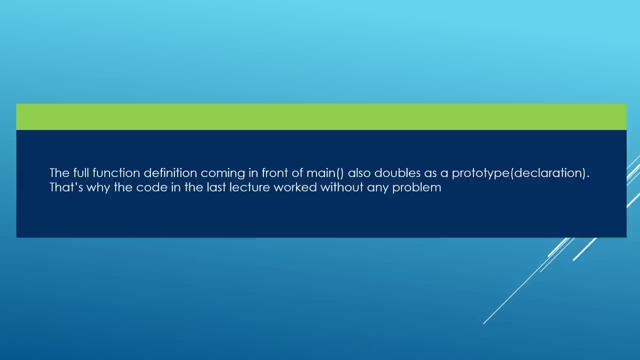 Well, if you put a function definition in front of the main function, that function definition is also going to double as a function declaration. That's why the code in the last lecture worked Okay. now that you have an idea about what a function declaration and a function definition is, let's head over to Visual Studio. 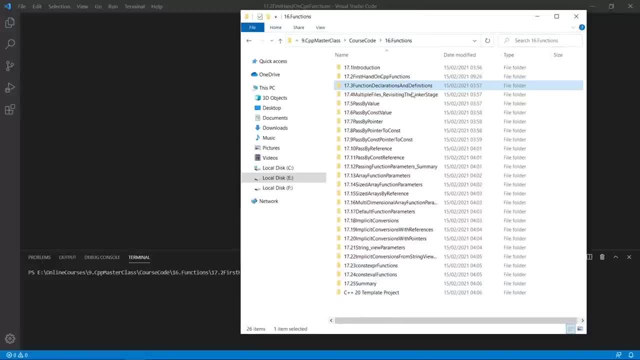 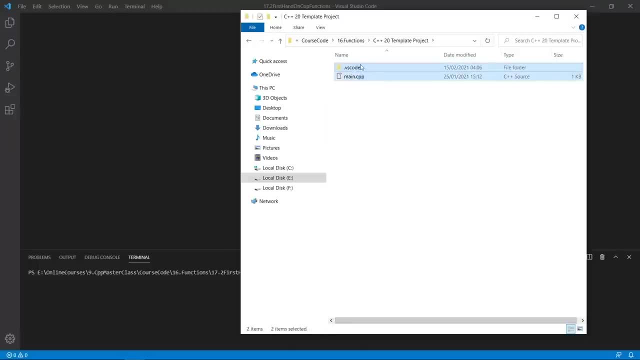 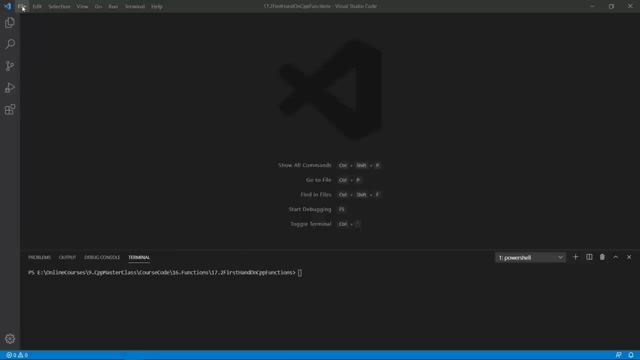 Code and play with us. Okay, here we are in our working folder. The current project is function declarations and definitions. We are going to grab our templates files, like we always do, we're going to put them in place and we are going to open this guy in Visual Studio Code. Let's do. 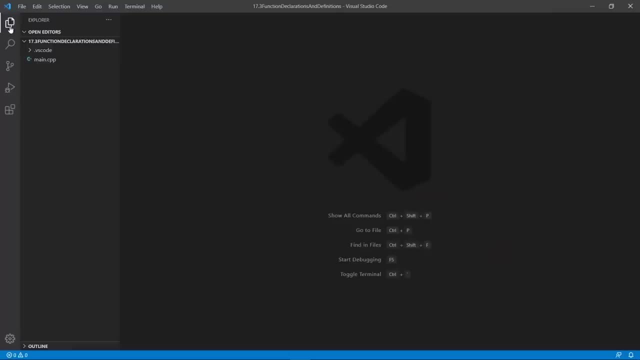 that We open this up, and we are going to open our main CPP file, clean it up a little bit and let's close this pane so that we have some breathing space. The first thing we're going to do is set up a maximum function. You already know how to do that. We're going to specify the return. 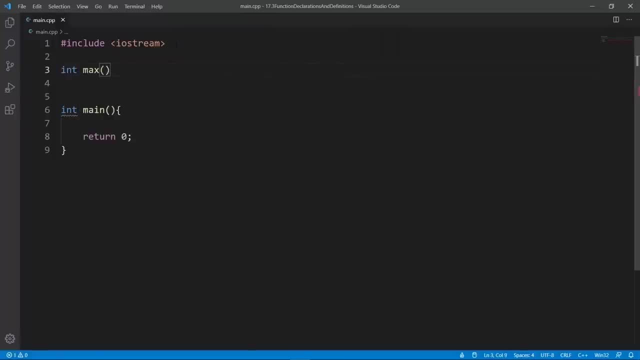 type. We are going to specify the function name and the parameters. We're going to take in it A and int B and we're going to go in and do whatever we need to compute the maximum between these two guys. We're going to say if A is greater than B, then A must be the maximum. so we're going. 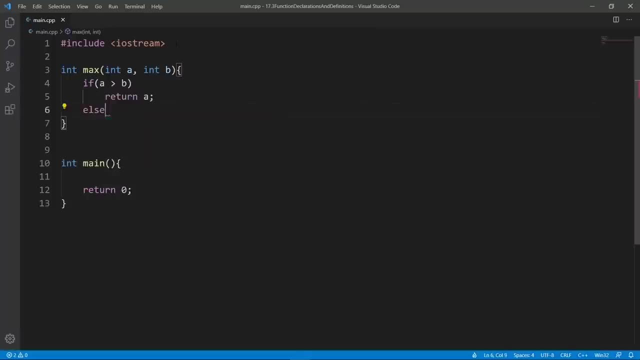 to return that, else we are going to return B. Okay, this is the function and it is really simple. We can go down in main and use it. so let's say int x and put in a five, for example, and let's say y and put in a two or a three, Put in whatever you want, and then we're going to set up. 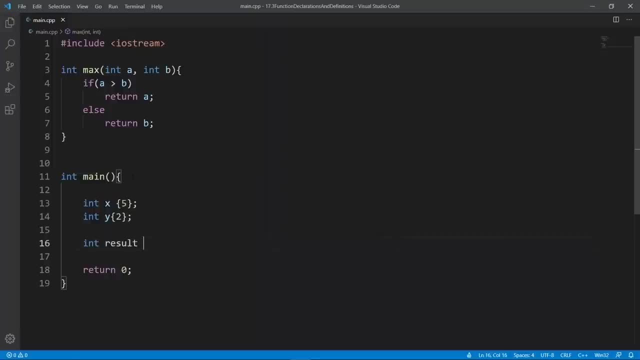 the reserved variable which is going to catch the maximum. I think we can do that, and what we're going to assign to this is whatever is returned from our function call. So we're going to call this function with x and y. so we're going to be computing the maximum between five and two here. 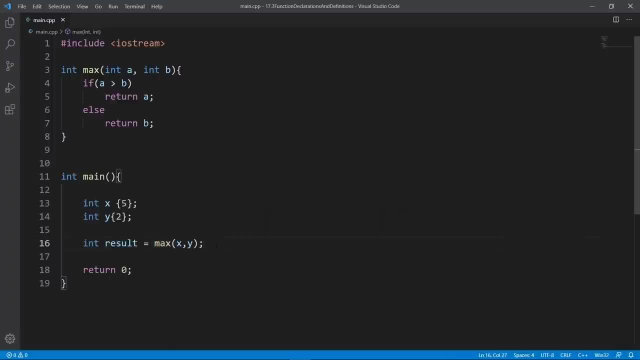 The maximum is going to be stored in this reserved variable and we're going to print it out. We're going to say std cout and we're going to say max. as result, This is going to do. Okay, let's try and build this and make sure it actually works. This is nothing new so far. It is everything we 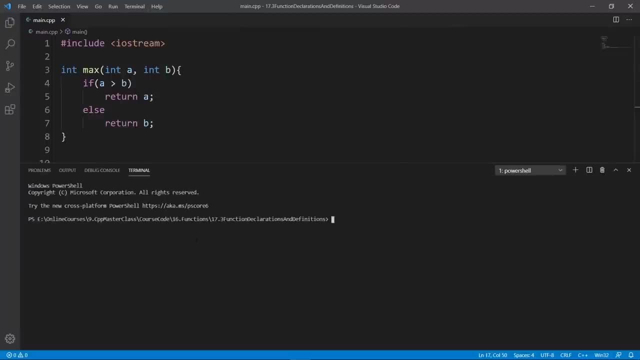 have done in the last lecture. Now the build is good. We can clear and run rooster. We're going to get the maximum as a five here. and if we try to change these things- for example make y a 12 and build again- 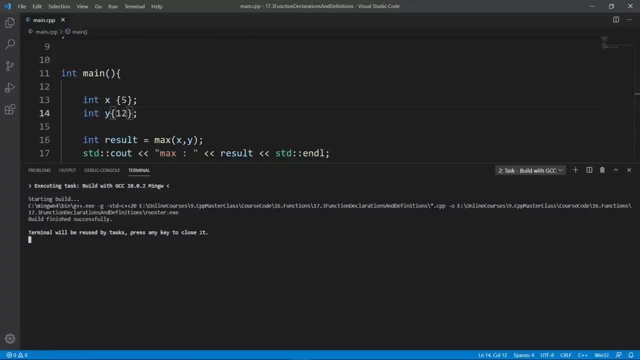 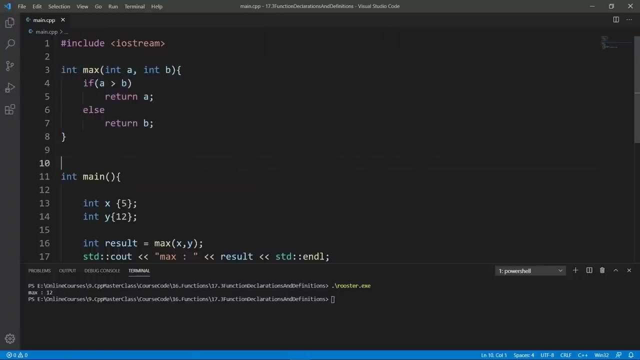 We're going to use gcc and we are going to clear these things and run rooster. We should get max equals 12.. This is all fine and dandy, but sometimes we don't really want to have the details about how our function works shown in front of the main function here and we can split our function. 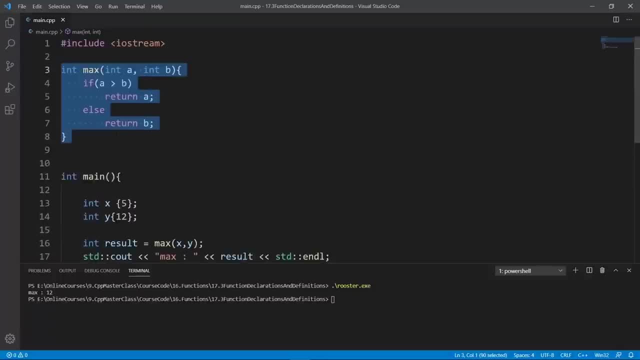 in two parts: A declaration and a definition. The declaration is really going to be the header part of the function, So we're going to use the header part of the function and we're going to use the function and that's going to be the return value, the name of the function and the parameter list. 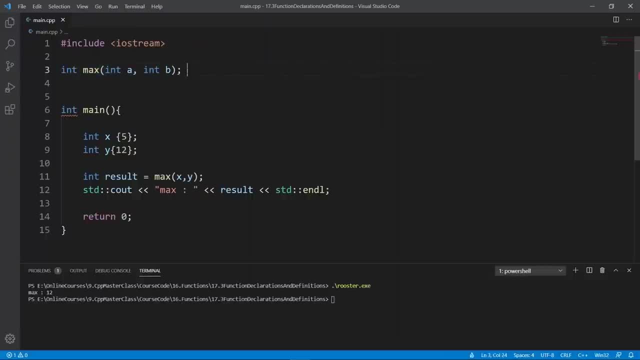 but to make it a valid declaration we have to put a semicolon after this. So this is our function declaration. Sometimes it is also called a prototype, and please make sure you understand the difference between a prototype and a signature. In the last lecture we saw that a signature was only made of the name of the function and the 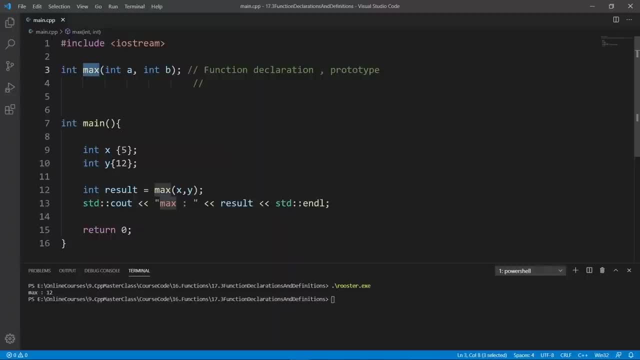 parameter list, but the return value was not part of the function signature, but the prototype includes all these guys, So signature doesn't include return type. Okay, so now we have our function declaration set up, we need to put in a function definition because if you try to compile, 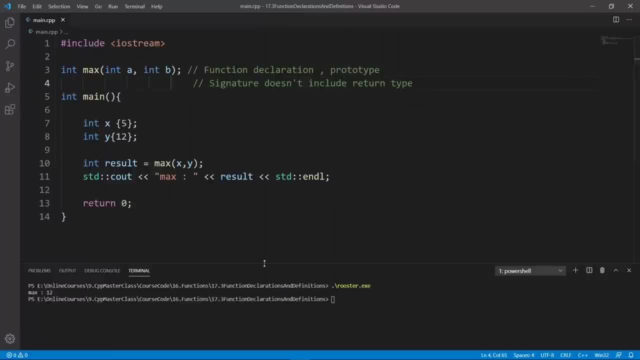 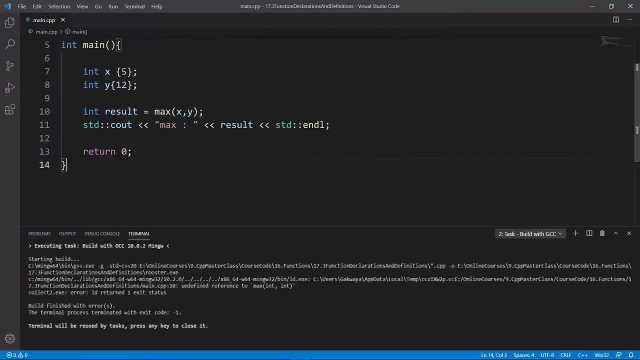 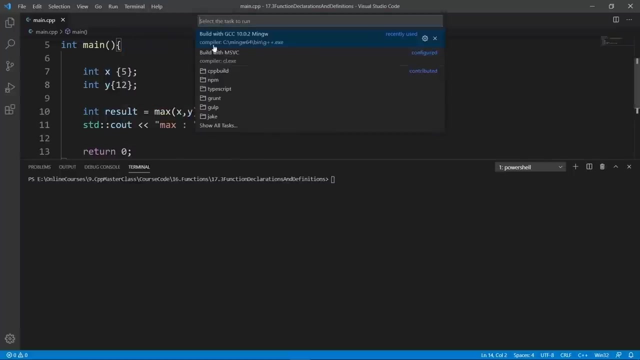 this program and link it. you are going to get problems. So let's try and do that before we put the definition. We can build with GCC. We are learning, so we don't have to fear breaking things a little bit. Let's clear and try to build with GCC and you're going to see we have a problem here. 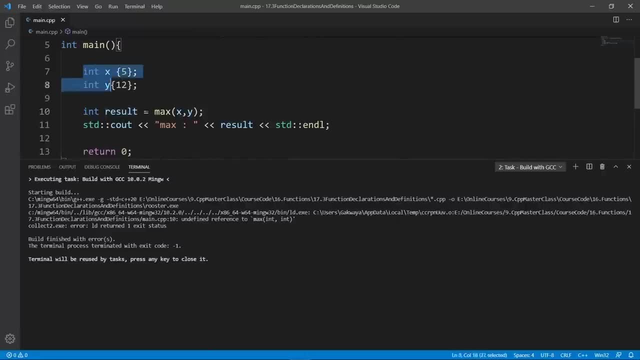 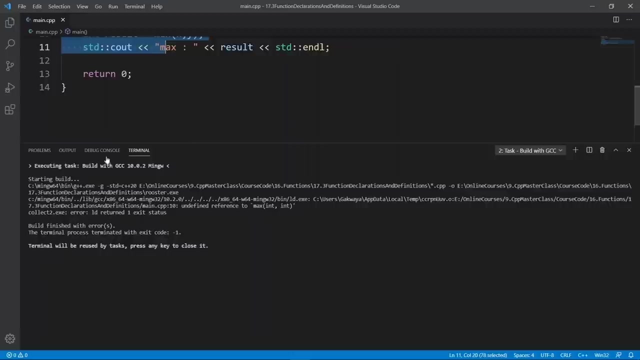 and what kind of problem we have. The C++ compiler is going to compile this program, but when we hit the link stage, I realize I haven't really talked about this in more detail, but we will do in this lecture. But the main problem here is that we don't have the definition of this function in place. 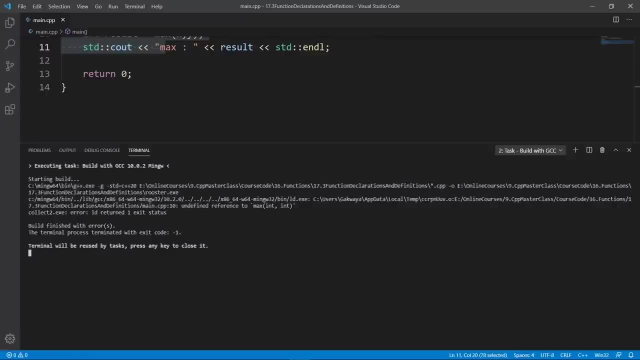 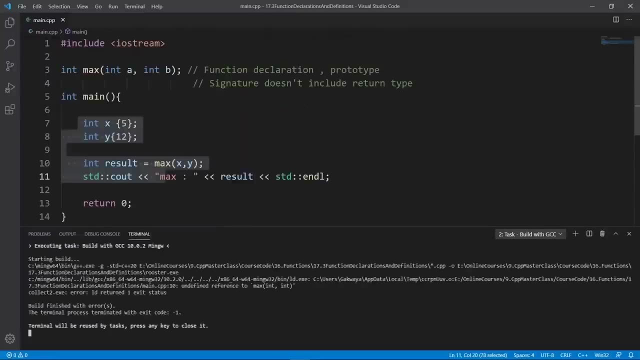 and the compiler is going to search for it and not find it. and you see that it is saying undefined reference to max. Okay, so it has seen the declaration of the function, but it doesn't know how the function does its job because we don't have a function body in here. So to really 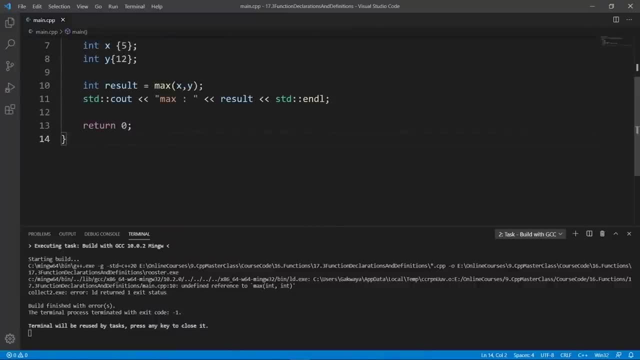 make this code work exactly as we want, we need to put in a definition, and the definition can show up anywhere in your C++ program. In this case, we're going to put that after the main function and the definition is really what we have been using so far as our function definition in the 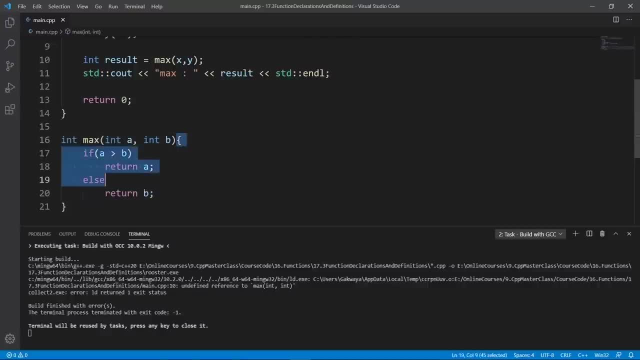 last lecture, but notice that it has the body information and now when the compiler tries to compile this program, it will know how the maximum function is computing its maximum, because we have all that information in here. This is our function definition and it shows up after main, in this case, and we can try and weld. 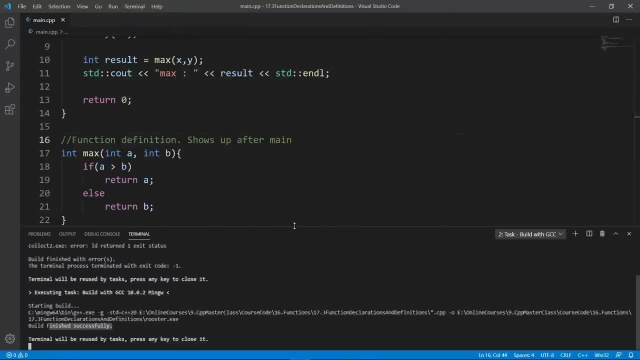 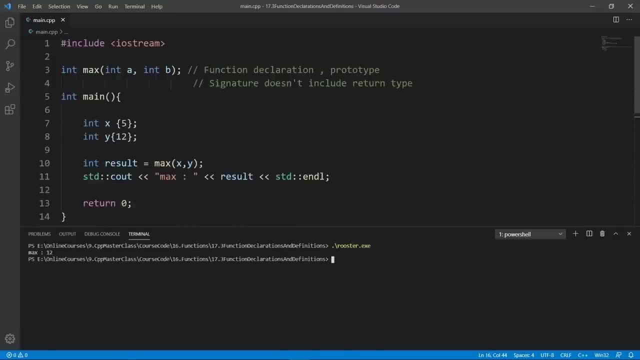 this and see if the weld is good. Now you see, the weld is good and if we try to run it we're going to get our maximum, exactly like we did when we had the declaration and the definition cramped up before main here. But hopefully now you can see that our program is much cleaner, because when you 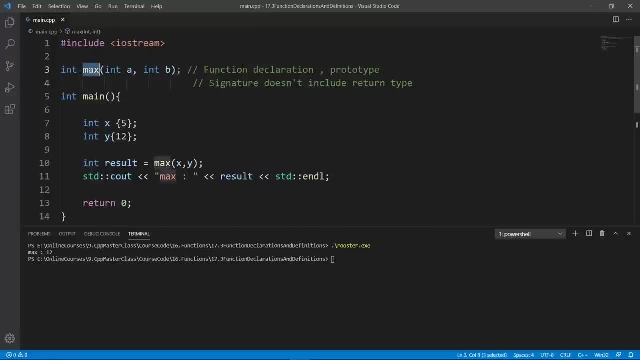 look at this. you know that we have a function called max. It's going to take two parameters, it's going to return something and it is called max, so it must be computing the maximum of these two guys. but we don't really care how this function does its job. 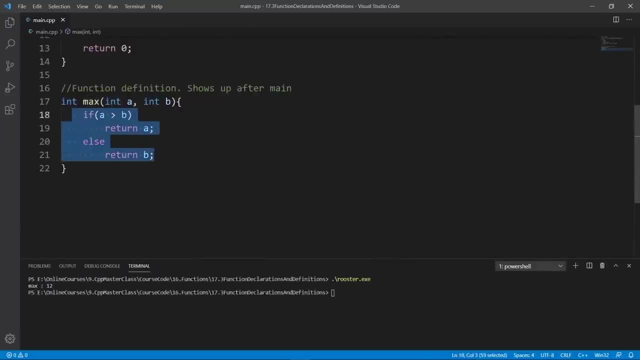 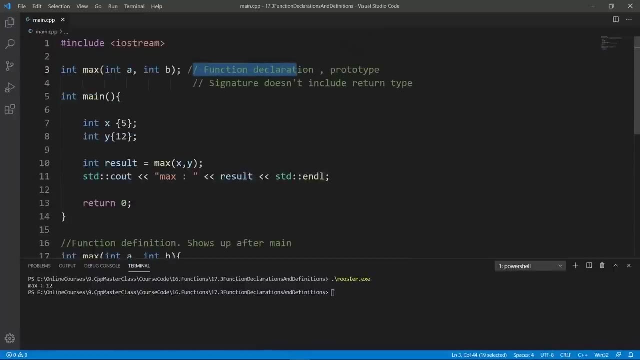 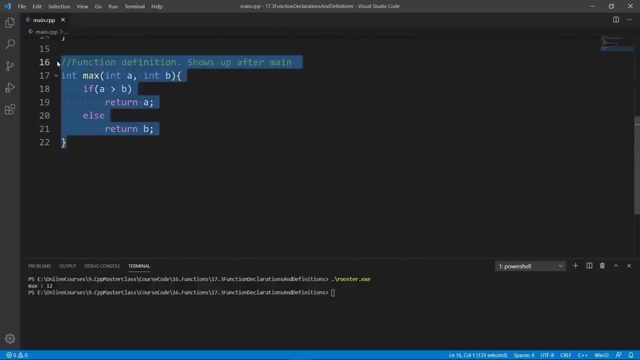 how it computes the maximum. here- and this is the main message here- we can split our function in two parts: a declaration and a definition. Okay, just to play around, we can also set up a minimum function. before we do that, let's set up its definition down here. we're just going to. 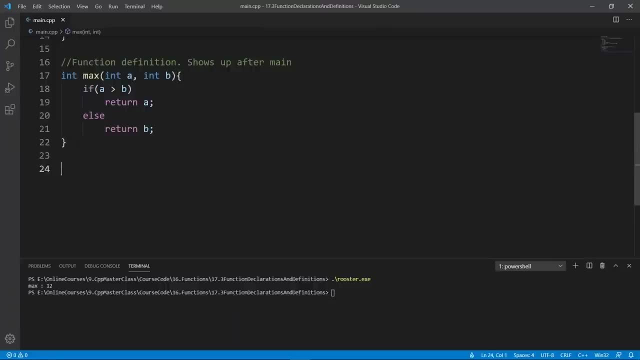 copy the maximum and adapt it. we're going to put a copy of that guy here. we're going to call it mem. it's going to take two parameters. it's going to return an end, but what we test for is if a is less than b. if a is less than b, then a is our minimum. if a is not less than b, then b must be. 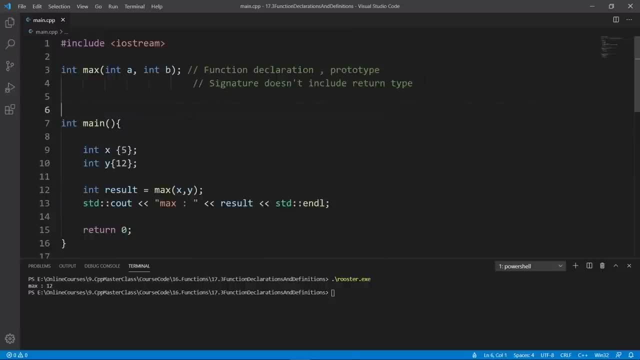 our minimum and we can put the declaration of this function on top here. so let's go there and say mem and say int a and int b, and now we can change the call here to say mean and it is going to compute the minimum. why not? let's do that? we're going to say min here and we're going to grab whatever is the minimum. 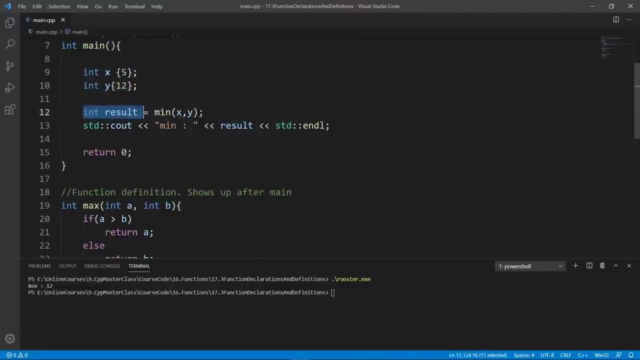 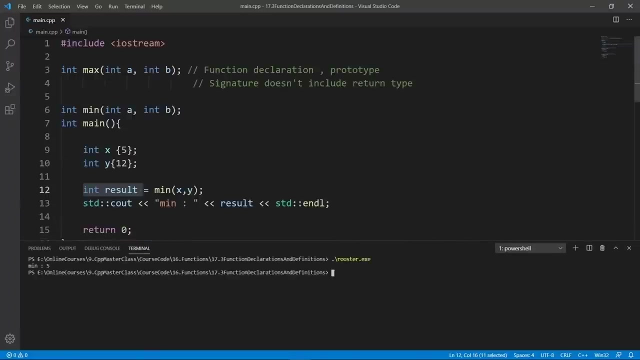 between x and y here, and that's what we're going to have in this result variable here. let's do that. we're going to try and use this. the build is good, so we're going to clear and run rooster. now the minimum is five. we are calling our minimum function. in the last lecture we also set up a. 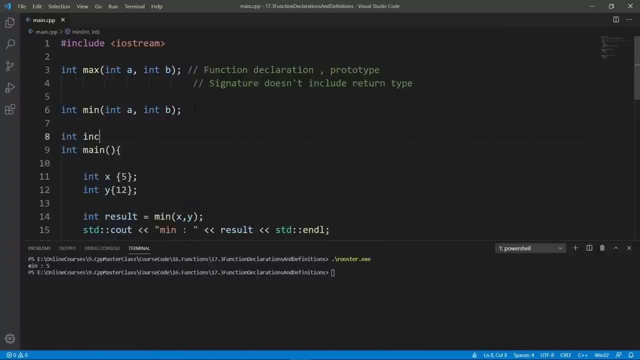 function to increment and multiply. let's try and do the same thing, but split that into a declaration and the definition. just to practice a little more. we're going to call this and malt and it's going to take a and b, n and inside, and we're not going to put the body on top here, we're going to put. 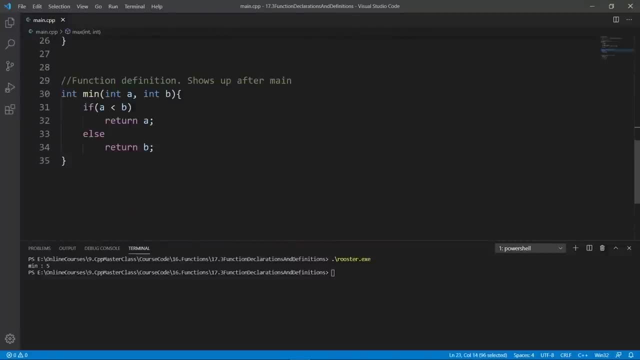 the body down with the other definitions that we have for all these other functions for max and mean here. so we're going to put in our body. it's really simple. so we're going to put a body in side, this curly braces, and we are going to return plus a, we're going to increment a and we're going. 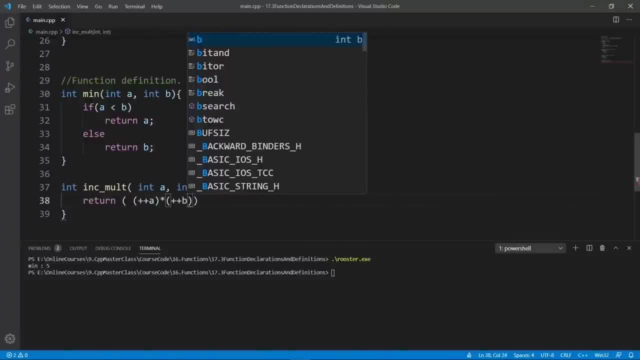 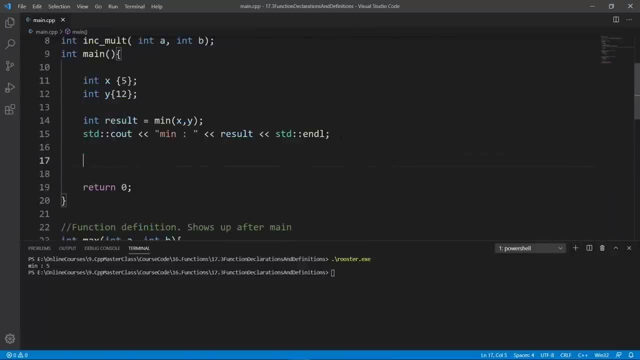 to multiply that with an increment of b and we're going to return that. i think this is going to be valid c++ syntax and if we try to call this function in main, let's do that, say, in malt, and we're going to pass an x and y. the program is going to just work fine. we're going to grab the. 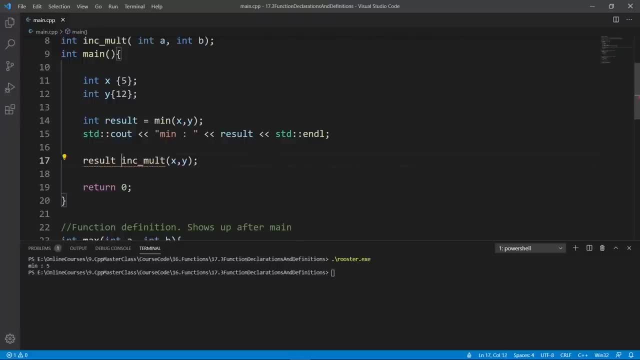 result and store that in our variable. let's do that and we can print the result and we're going to say result here: this is going to do and if we bolt and run this program, we're going to see the output here. let's see what we get. the result is going to be 78 because if we increment a 5 it becomes a 6. if we increment y. 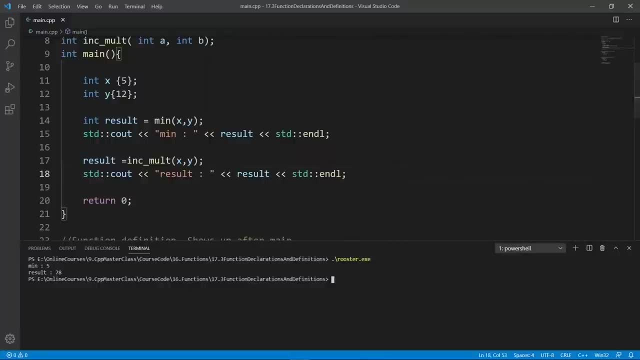 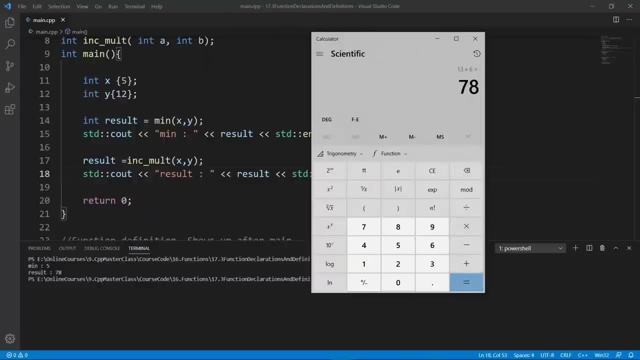 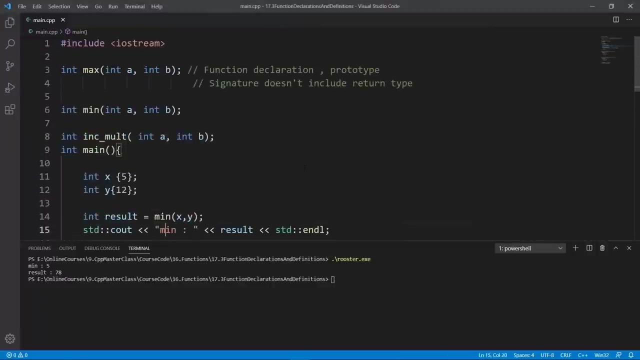 we're going to get 13. 13 times 6 should be 78. let's make sure we're going to bring up the calculator. let's do that so that you know that i am not making these things up. 78. so our program is really working like it should, and this is the main message here. 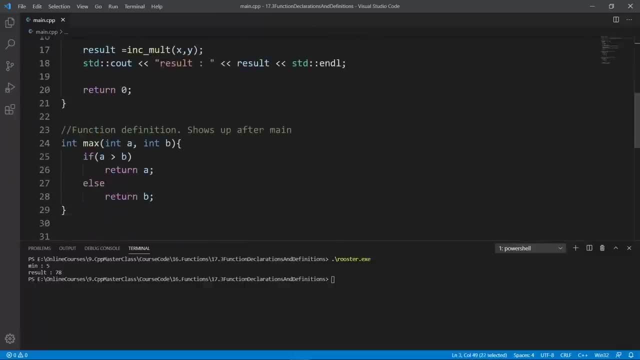 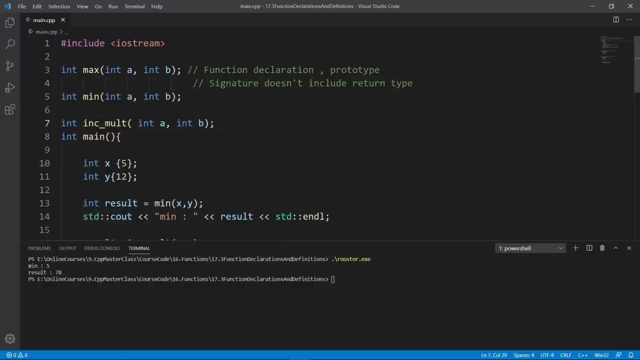 we can really split our functions into a declaration and a definition, and that's going to make our programs much easier to work with and read. one thing you should know is that the names of the variables aren't really important in function declarations like this. so, for example, we can take out the a and b here, or we can take out all the variable names in our 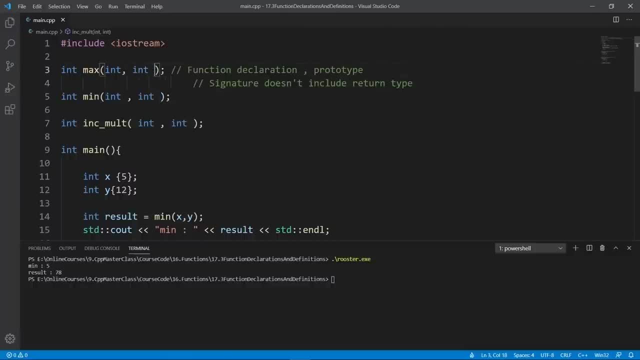 function declarations. let's do that. and you might think: is this program going to compile? well, i hate to break it to you, but it is going to compile. so let's world. with gcc, you're going to see that the world is good. so the function header or declaration doesn't really care about the variable names. 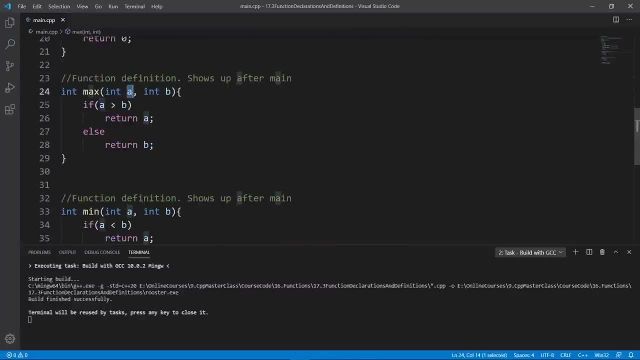 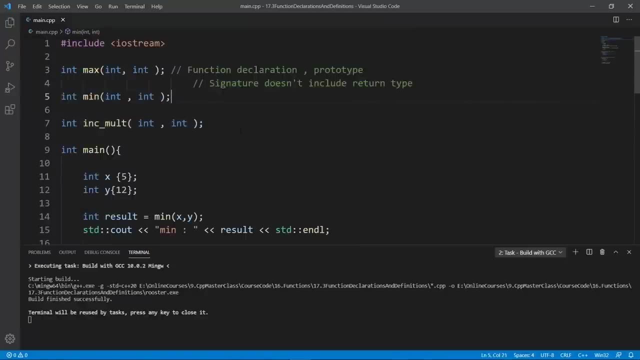 in the definitions. we care about these variable names because we are going to be using them in the bodies. but if you want, you can leave them out in your function declarations. but i like to keep them in place because i like my functions to be self-documenting. if somebody looks at this, they 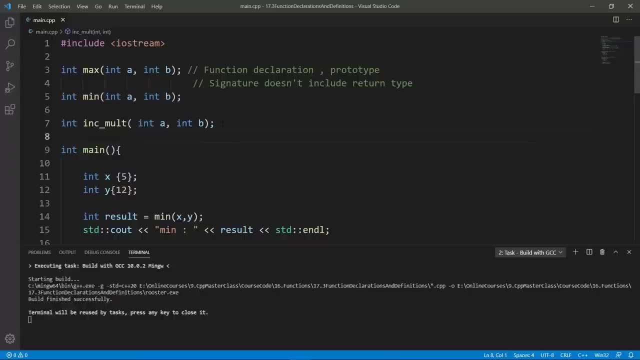 will know the variable name here. but if you really want, you can leave the variable names out and it is going to work pretty well. this is really all we set out to do in this lecture. i hope you found it interesting. we are going to stop here in this lecture. in the next one we're going to see how we can split our 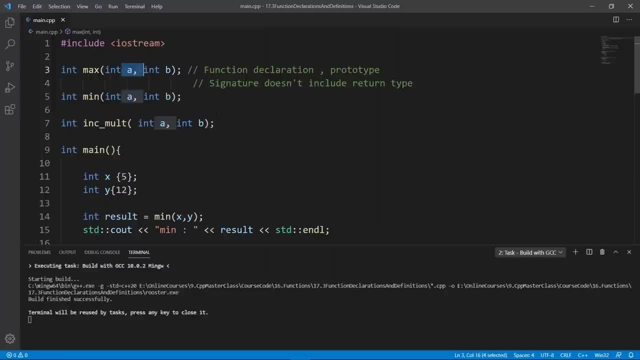 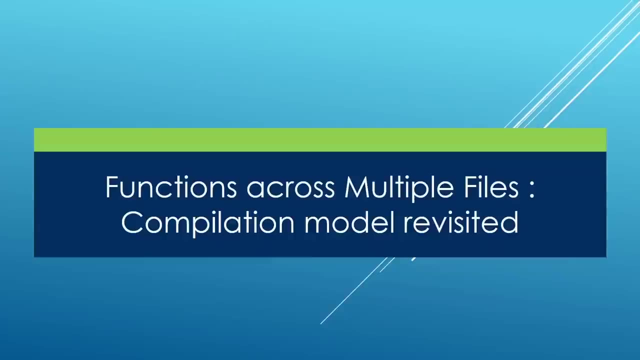 programs in multiple files. now that we know how to split into declaration and definition, go ahead and finish up here and meet me there. in this lecture we're going to revisit our c plus plus program compilation model. along the way, we are also going to see how we can work. 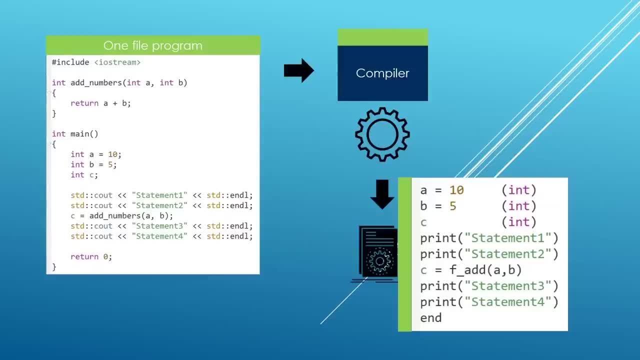 with functions across multiple files. if you remember, our compilation model looked a little bit different than the one we saw in the previous lecture. we are going to see how we can something like this. you have seen this slide a lot of times by now. what it describes is what 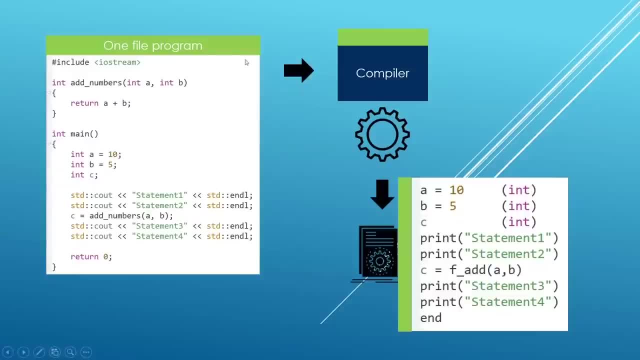 happens when we compile our program. the moment we run the compilation command, our c plus plus program, which lives in the main cpp file by now, is going to be passed through the compiler. the compiler is going to process it and it is going to come up with a binary executable. 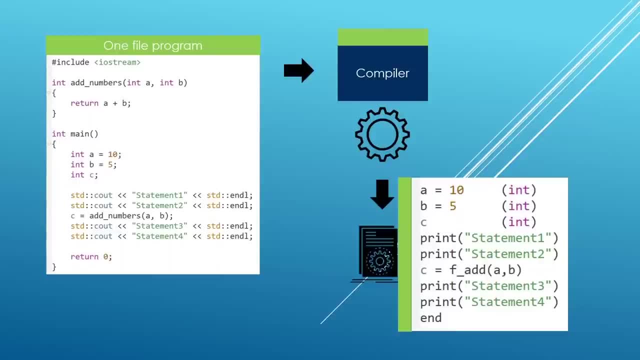 that is mostly called rooster in this course, and when we execute this rooster file, or binary file, we're going to get the program to run. the program is going to be executed instruction by instruction when it is loaded by the operating system and we are mostly going to see the output. 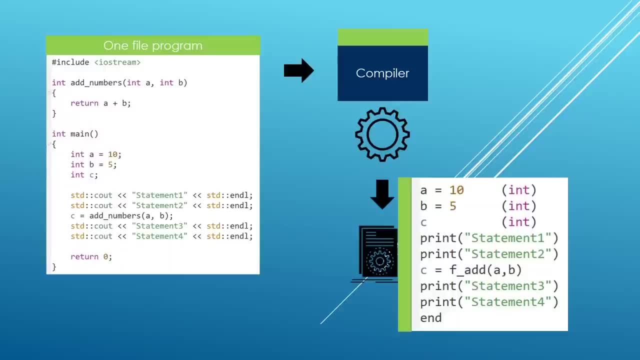 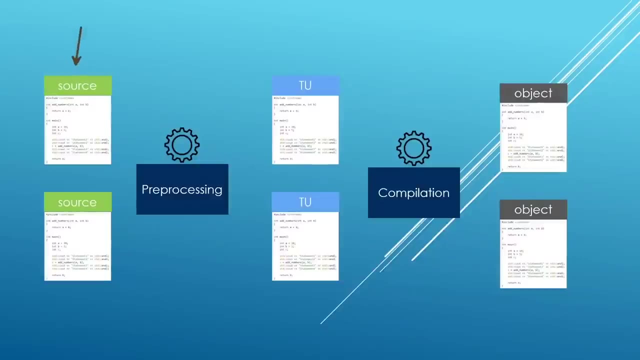 of that program on the terminal in this course. this is the compilation model we know, but now what we want to do is zoom in on this compilation part here and see what really happens under the hood. we are going to suppose that we have our program, which is made of a lot of 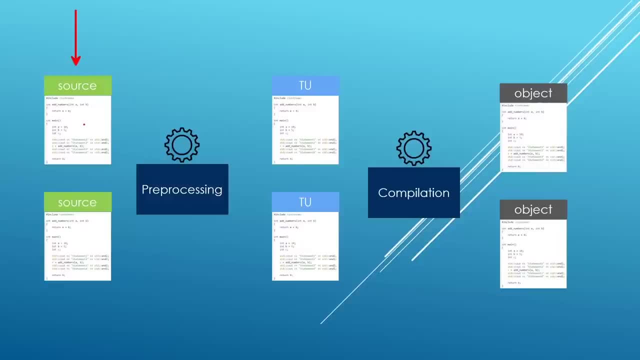 source files, as we have here on the left. suppose we have two, three or five source files, unlike what we have so far, which is one file, the main cpp file. when you compile such a program, you're going to go through a stage called preprocesing, and what this is going to do, it's going to look for your 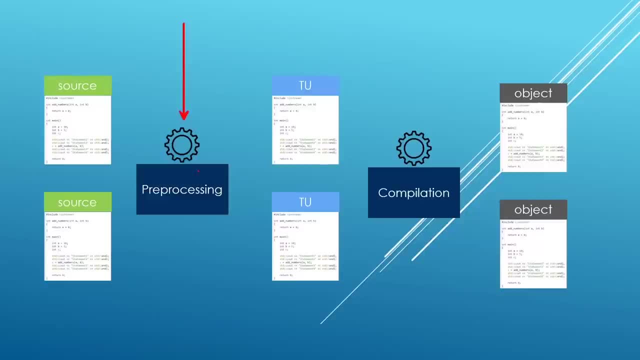 include statements and it is going to take whatever file you are including and it is going to paste that in place. So, for example, here you see what I am using here- compressor import components- and what I am pulling this out. We areandoq Fish. You can see that they are working You. 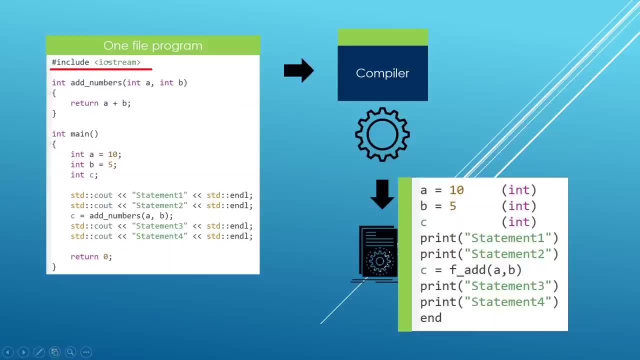 we have an include io stream statement when the pre-processing stage is run. this include statement is going to be replaced with whatever we have in this io stream file here, so this is going to be wiped out and we're going to put in the content that we have in io stream in this exact place. 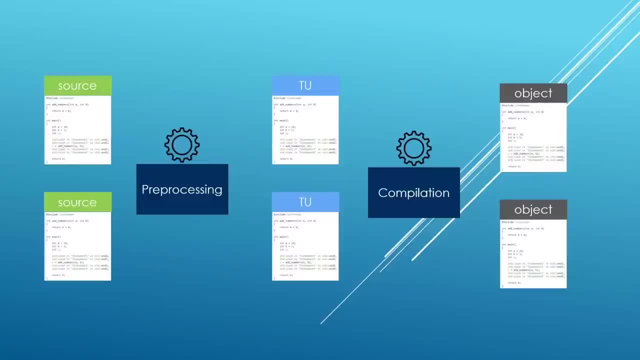 where we have the include statement. i hope this is clear. so when we go through pre-processing, we're going to have a version of our source files with the included parts put in our source files. we're basically going to go copy everything in that file that we include and we're going to paste. 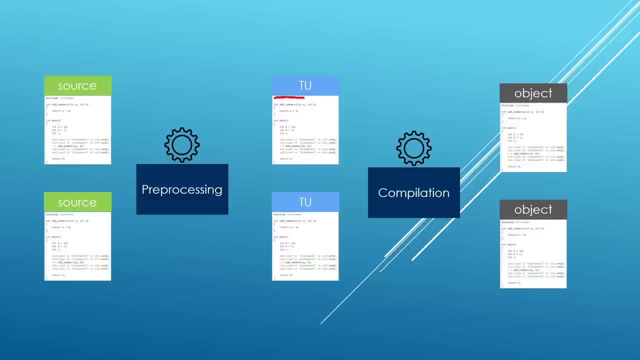 inside our new files here that we're going to be referring to as translation units. by now these are translation units in a c++ program. once you have these translation units, then you're going to compile them. they are going to go through the compiler. the compiler is going to generate what we call an object file. 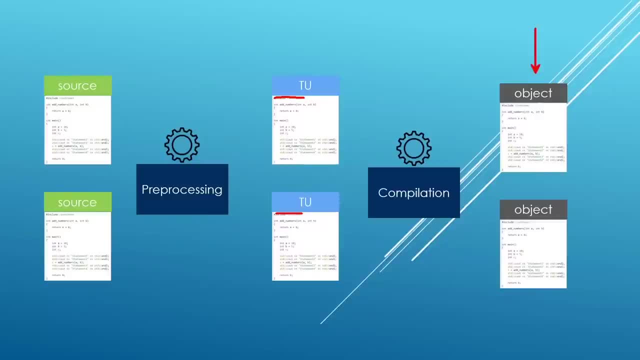 and this is a binary representation of the content you have in your translation unit. so each translation unit is going to generate one object file and, for example, if you had 20 translation units in your program, you're going to have 20 object files once we have object files. 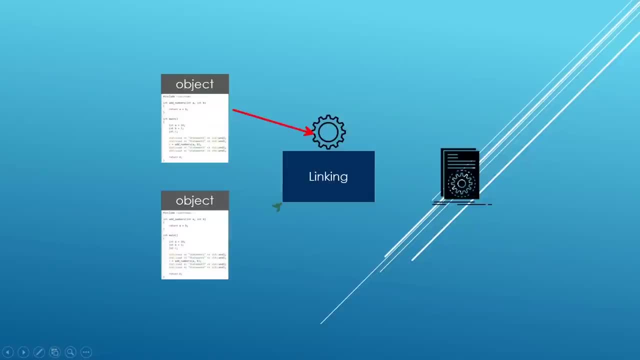 they are going to be processed by what we call the linker, and at the linker we're going to have a single binary file which is something like this, and that's basically going to do with the sequence of all these object files that are going to be placed. so the linker is going to stitch them. 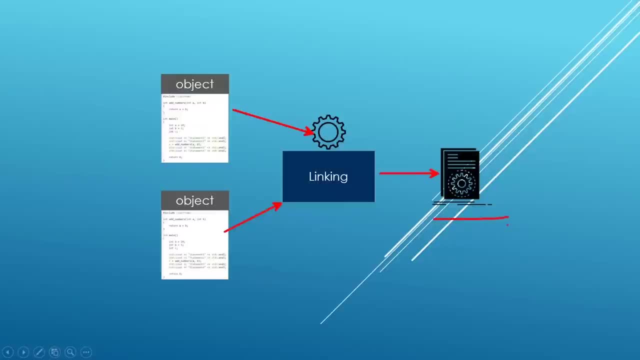 together and have one single binary file out of all these object files. so we're going to have something like this, and this is basically going to be our binary that we can run on our target operating system. so by now you see that our compilation model has expanded to contain three. 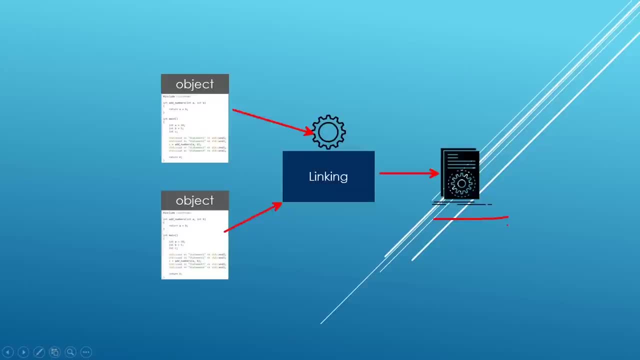 phases. we have pre-processing, compilation and linking. now you might be asking why am i showing split our program across multiple files. some of those files are going to matter on the compilation phase and some of those files are going to matter on the linking stage. So we really need to make a 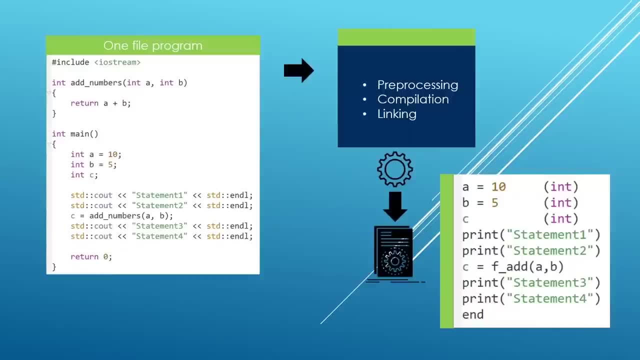 clear distinction between compilation and linking here. Okay, this should be a more complete compilation model to go by for now. Now that we know about this compilation model, we can look at how we can split our program across multiple files. Suppose we have three functions: One we can. 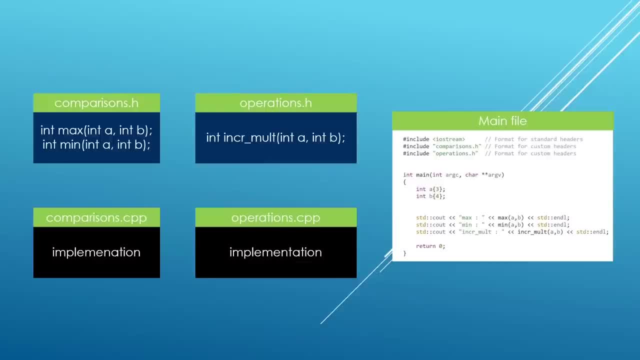 use to get the maximum of two numbers called max, a function called min we can use to get the minimum between two numbers and a function we can use to increment and multiply, like we have seen in the last lecture. Now the two functions, max and min, are going to live in their own file and that file is 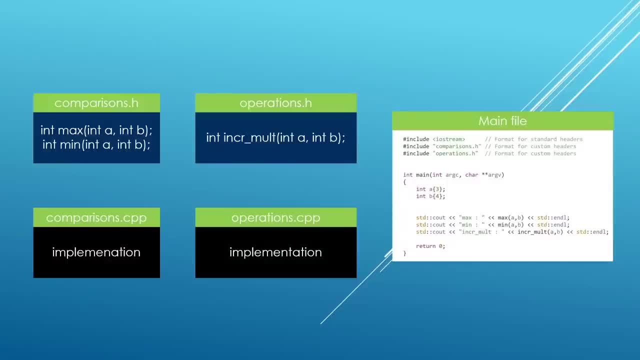 going to be split in two files. We're going to have a header file and a cpp file, which is going to contain the implementation In the header. what we're going to have is just a prototype, and we are going to set up our code in a way that. 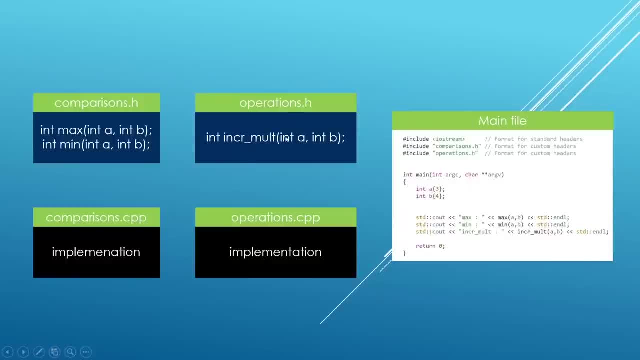 our anchor malt function here is going to live in its own file. We're going to split that in two files, so we're going to have a header file called operationsh and we're going to have an implementation file called operationscpp which is going to contain the implementation of this function here. 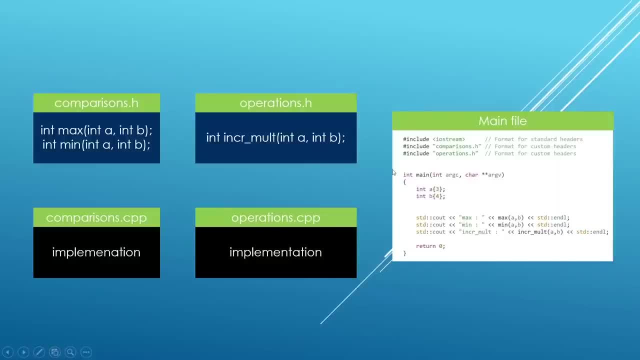 When we hit the main file. what we're going to do is nothing special. we're just going to include the headers And we are going to use these functions like we have been using them all along. If you look, on the first line, here we are calling max. on the second line, we are calling min and on the third line, here we are calling. 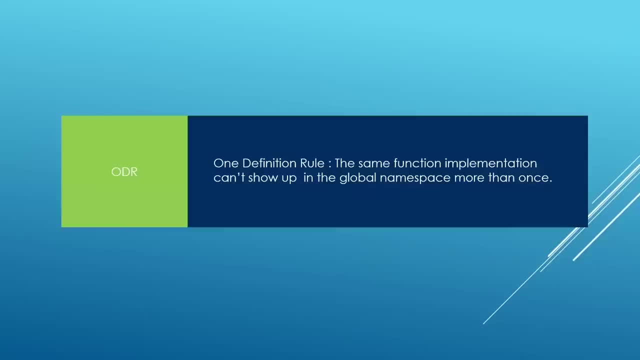 anchor malt to do whatever it does. Okay, when you start splitting your functions between definitions and declarations, remember the one definition rule and this says that you can't have a function defined multiple times in your entire system. If you do that, the linker stage is going to find those two functions and it's going to not know which. 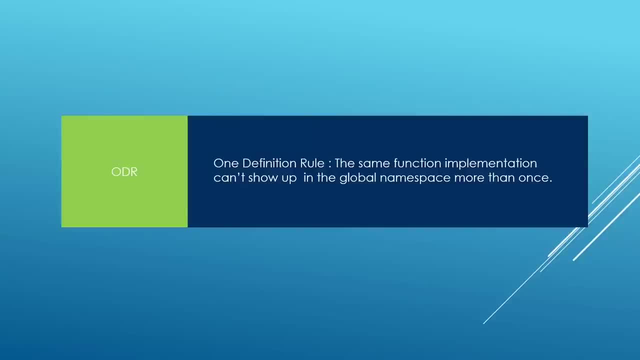 one you really want to use and you're going to get a linker error. We're going to see that when we hit Visual Studio Code in a minute. Another thing is that you know that your definition can really live anywhere in your code. The linker is: 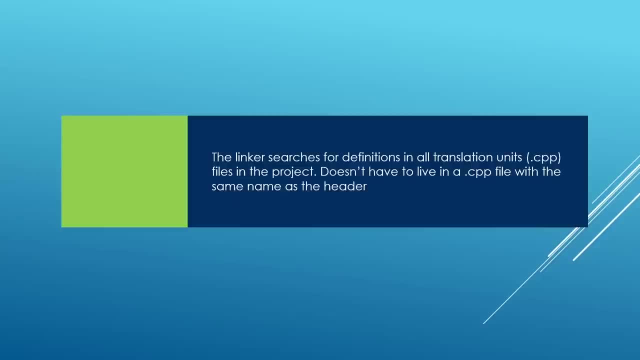 smart enough to parse your entire project, looking for the definition for whatever function it's found in your source code, And it's going to keep looking until it finishes looking in all translation units and when it doesn't find the definition, it's going to give you a linker error which is probably going to say undefined reference to something and 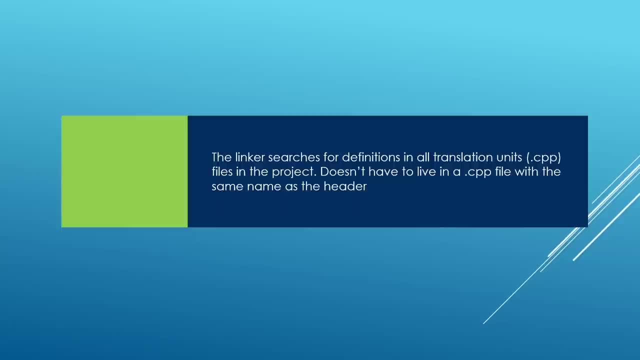 we're going to see an example of this in a minute. Okay, now that you know about this updated compilation model and you have an idea that we can split our functions across multiple files, we're going to head over to Visual Studio Code and play with us. 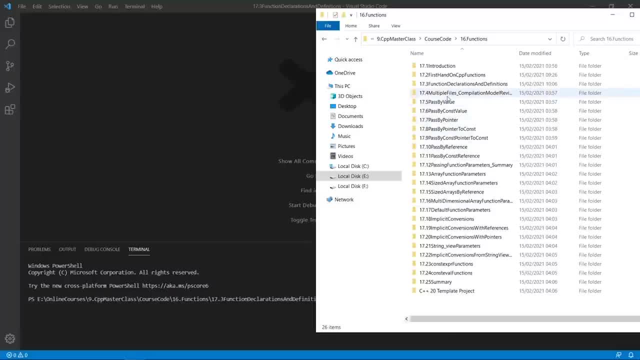 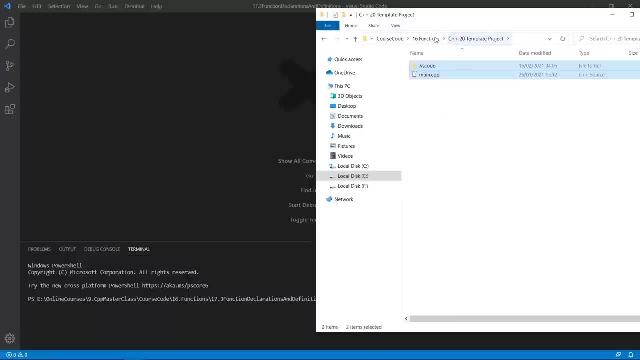 Okay, here we are In our working folder. the current project is multiple files. here We're going to grab our template files. let's copy that and put that in the project of interest, and we're going to open this in Visual Studio Code. 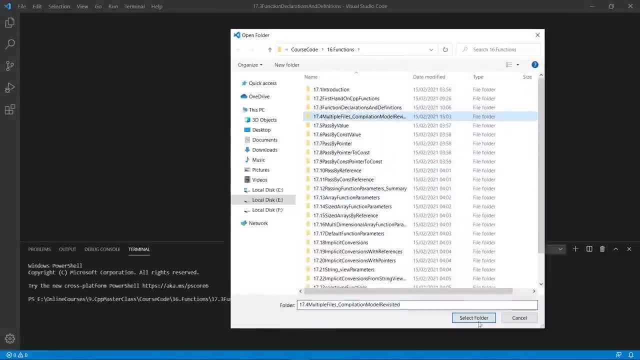 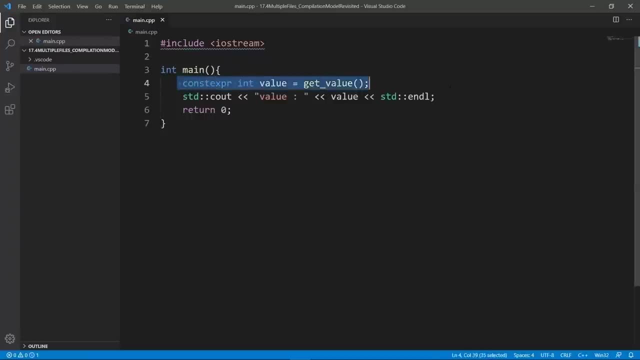 Let's do that. We're going to open the folder, we're going to choose the project and open it, and we are going to open up the main CPP file here and clean it up a little bit. We are going to set up a maths function. 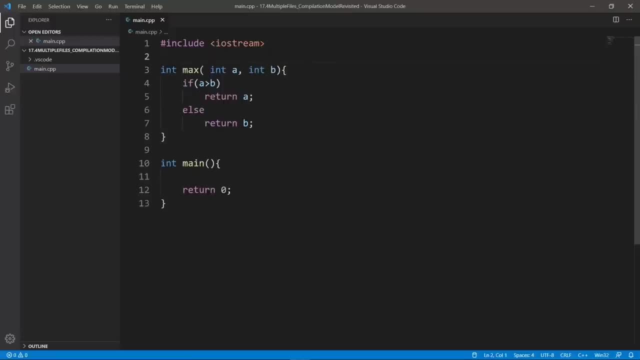 And remember, the function has to show up before it is used somewhere and we are going to split this into a definition and a declaration. I think we already know how to do that, so let's do that. We're going to put a definition down here and we're going to change what we have on top here into a declaration. 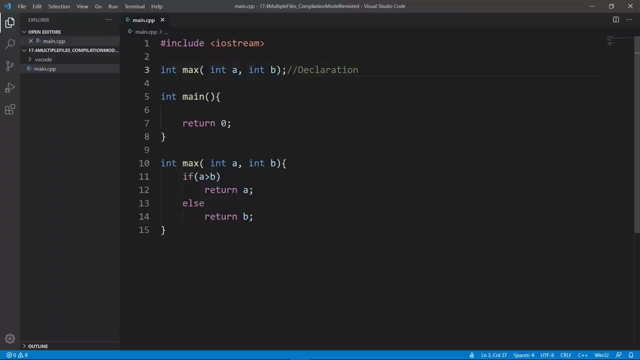 Let's save that to be super clear. and what we have down here is a definition and we can call this function. We're going to set up a variable, which is going to be the function, and we're going to call it a function. 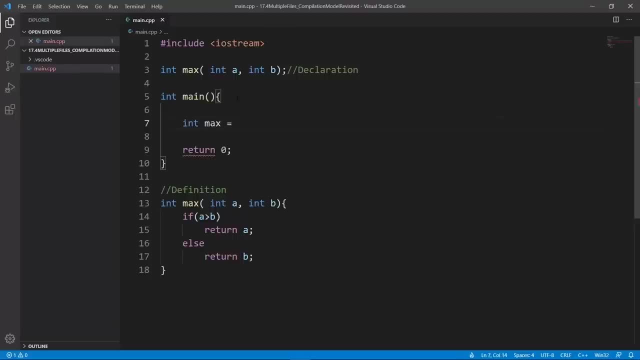 Let's do that Now. we are going to take this function here and we're going to set it to be a function. Now. we want to find the maximum between 34 and 56,, for example, and we're going to print this out. 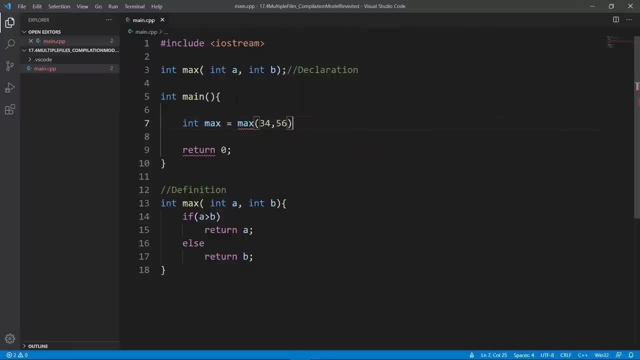 We're going to say: max is the maximum, And if we will then run this program, let's use gcc to do that. We have a compiler error here. What is that? We need a semicolon, not a colon here. I think the squiggly line is now going to be there and we need a semicolon here. 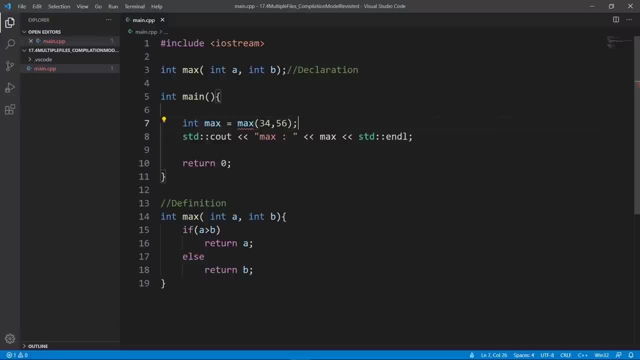 And we are going to print this out. So, now that we have the function, that is going to be here, And then we are going to change it to Max, Let's do that. going to go away and our things are named the same way. the compiler is not going to like it. 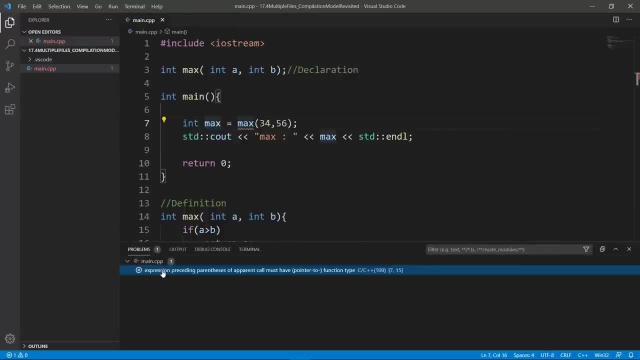 let's bring up a terminal so that we see our problems. tab expression preceding parentheses of varical must have: ah, okay, the problem here is that these two guys, max and max, are called the same, and this is going to confuse the compiler a little bit. so what we're going to do? 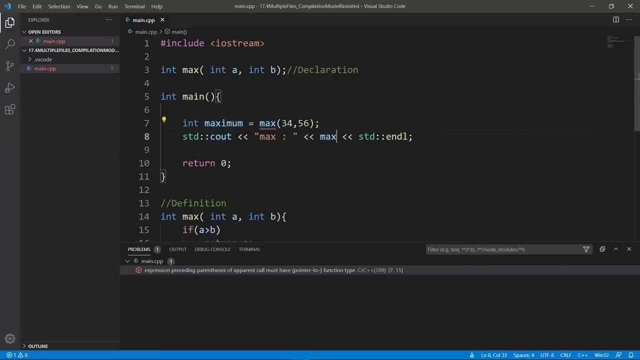 it's called this maximum. no big deal here and we're going to do maximum here and the compiler is going to be happy. now we can compile and I've boiled this program. boiled is good and if we run it we should get our maximum printed out. let's see that the maximum is. 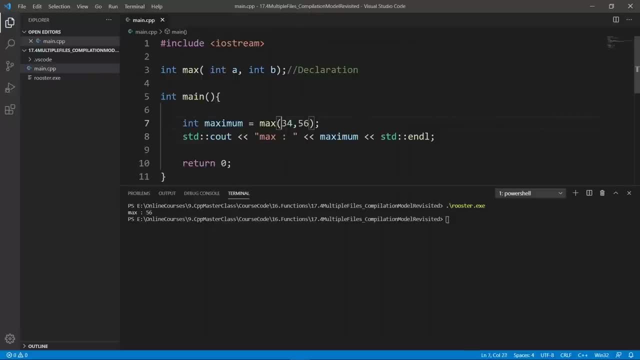 56 and if we change 34 here to be 134 and boiled again, we should grab that as the maximum and we can compile and I've spoiled this program. boiled is good and if we run it we should maximum- let's see if that's the case here- run the program. the maximum is 134, so this is working. 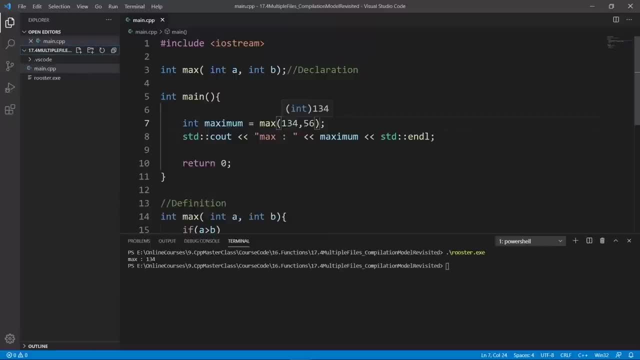 exactly as we want. the next thing we want to do is to split this function across multiple files, so we're going to set up two different files. one is going to be a header file, the other is going to be a cpp file, and you have to follow this structure in c++. so we're going to go on the 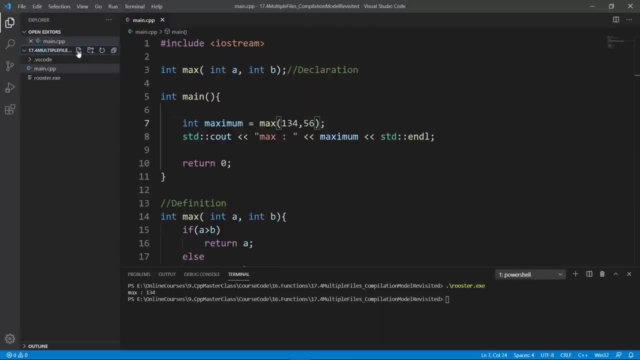 left here and add a new file. in visual studio code, you can click on this little icon that says new file to create a new file. once you do that, you're going to be given this little window in which we can type the name of the file we're going to call this. compare dot h. it's going to be our. 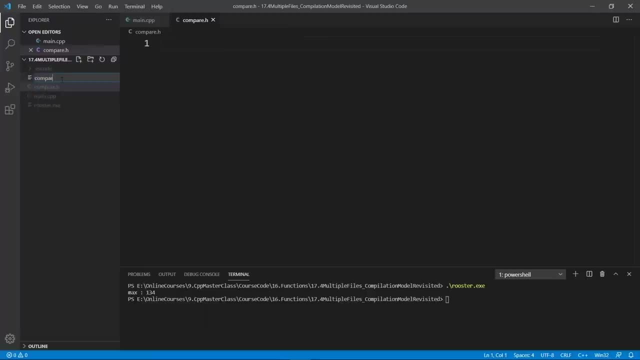 header file and we're going to add another one which is going to say compare dot cpp. okay, our two files are going to be compare dot h and compare dot cpp and they are going to contain our functions to compare stuff. so we're going to have in a function. 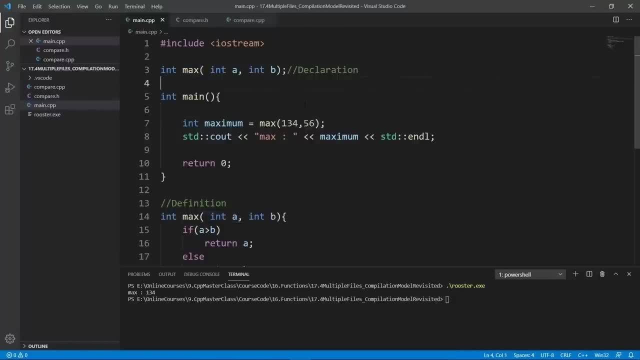 called max and another function called men for computing the minimum. let's go there and actually do that. we're going to move our declaration in the header file, so your declarations are going to be living in header files and we're going to grab our definition and move that in another file. 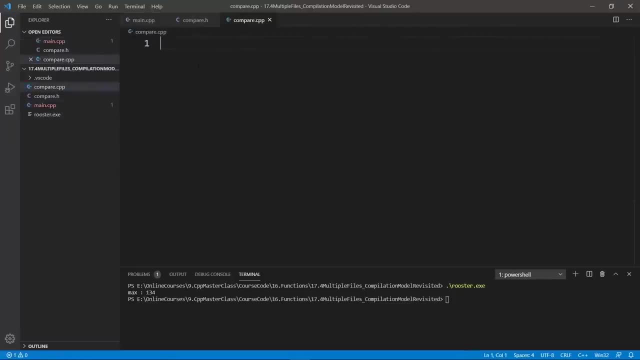 called compare dot cpp, so i'm just going to cut it out and paste that in compare cpp here. once we do that, we're going to go back in main and see that we have a problem. now the main function doesn't know what this max function is because it's not declared anymore, and if we're trying to compile our program we're basically going 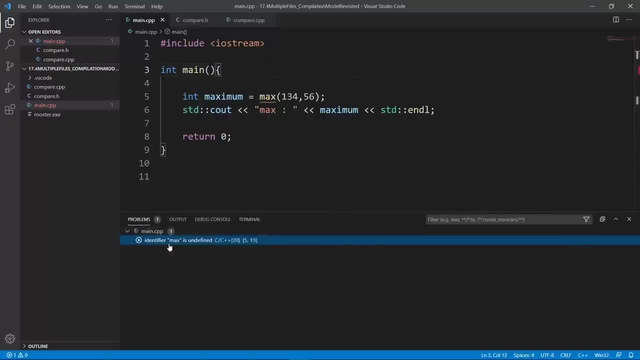 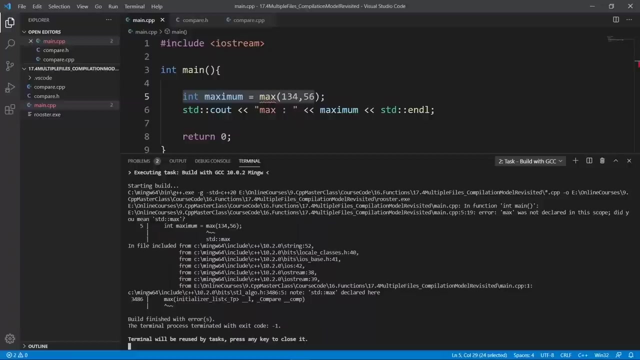 to get the same error we see here in visual studio code. identifier max is undefined because it doesn't know what this function is. if we ignore this and try to world, let's do that. we are a lot learning, so no big deal here. we're going to get an even much weirder error, but the message is going. 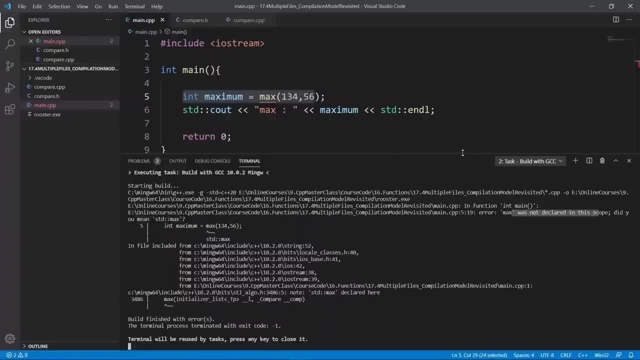 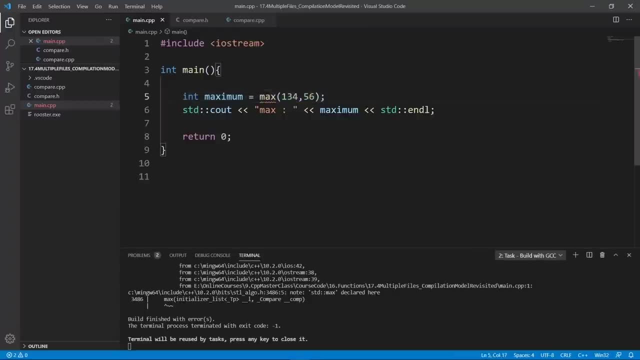 to be the same. max was not declared in the scope, so the compiler doesn't know what to do with whatever we typed here. but there is a way. in c plus plus we can solve this problem by including the header that contains our declaration for the function that we are using here. we can go back in main. 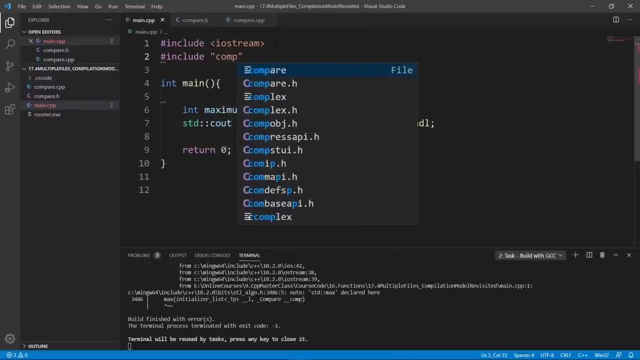 and do that and we're going to say include and we're going to say compare dot h. that's going to bring in our header and if you wait a minute, you're going to see that the squiggly line is going to go away. so what happened? the preprocessor is going to come in. 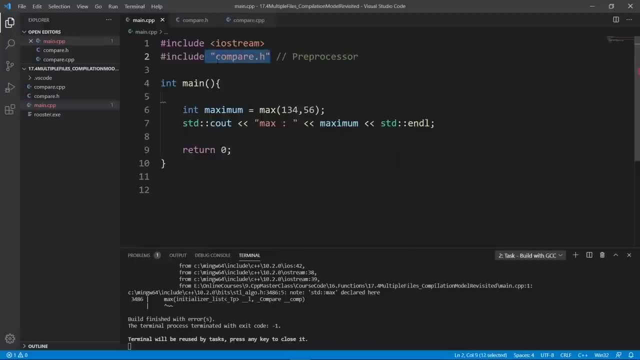 and copy whatever we have inside compareh. it's basically going to go in compareh, copy everything we have in here and come back in main and paste all that in the place where we have the include directive. here this is called an include directive or an include preprocessor directive. this is what the 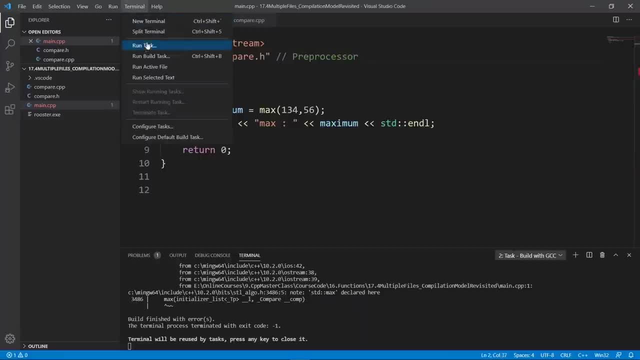 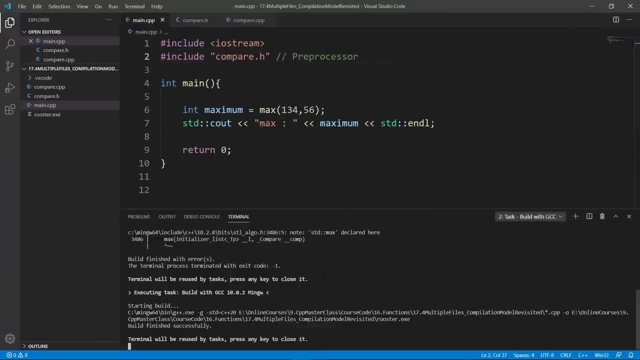 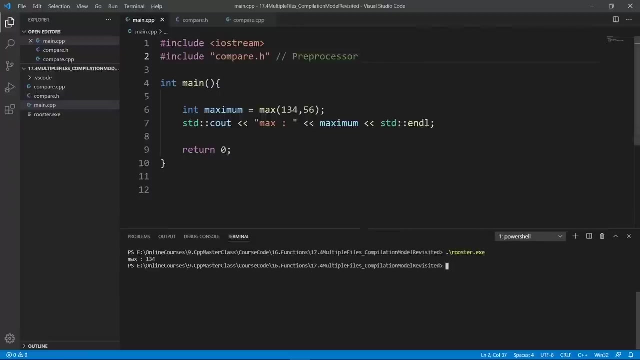 preprocessor is going to do here and now. if we try to build this program, let's try to do that- we should be fine world finished successfully and we can run our program to see the maximum printed out. let's run roaster. maximum is 134 now everything is working. let's add another function here, because 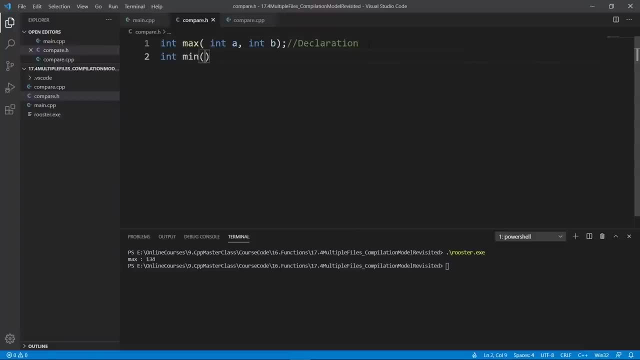 just having one function is really boring. so we're going to put in a main function. it's going to take int a and into b and we're going to go in the cpp file and put in another definition for the minimum function. here we're going to call this man. 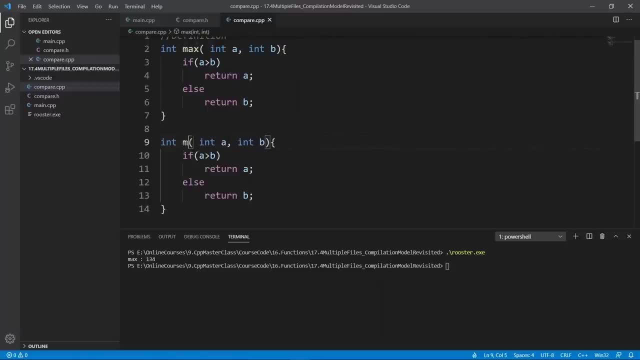 let's do that, let's call this man and we're going to test, for a is less than b. this is going to give us a minimum and now, if we go back in main cpp, we'll be able to use our minimum function because it is brought in also by this preprocessor directive we have here, so we can go down and 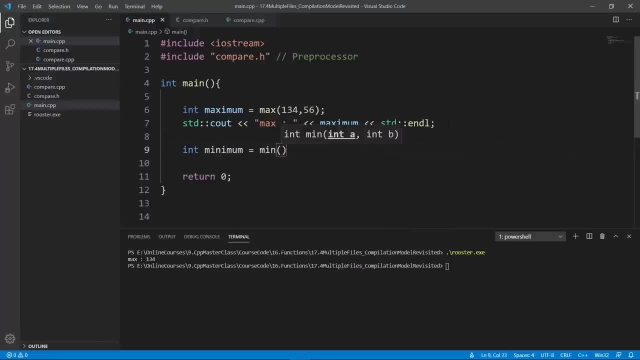 say and minimum, and we're going to say men, and let's grab 146 and 23, why not? and we're going to print the minimum here and we're going to build this with gcc. the book is going to be good. if we run this, we should see both the maximum and the minimum from these calls we make here. 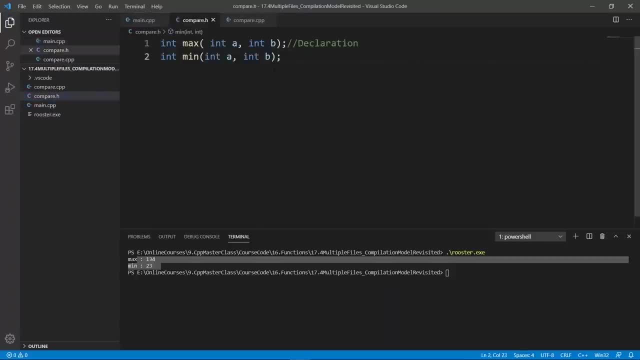 by now, you should have an idea about how to split your functions across multiple files. you should also know that you will have to include, whatever header contains, the declarations for the functions that you want to use. another thing i want you to see is that the definitions for your functions 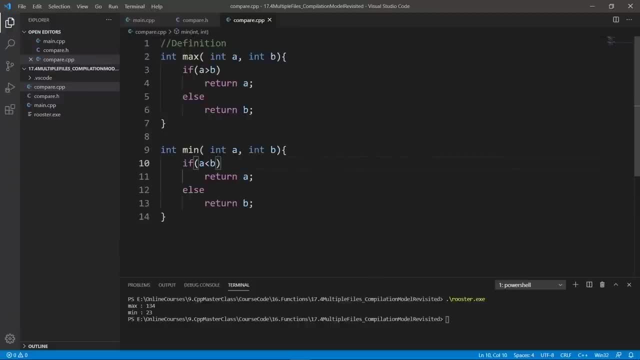 don't have to live in a file that is named the same as the header file. for example, here our header file is called compare and compare the header file is called sliced header file, and the header file right here is also Joshua head. in this case we want to use cross실 to say these are heading, Meanwhile, go ahead. 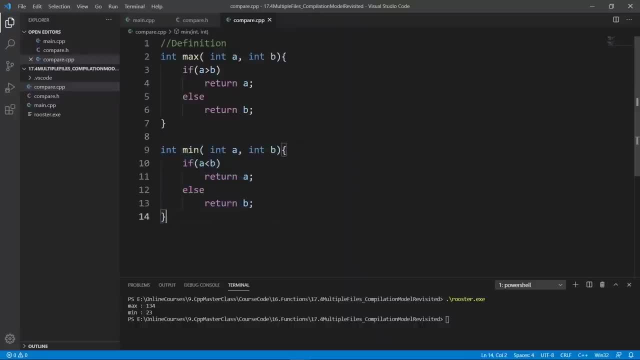 cpp contains our definitions, but the definitions don't have to leave here. they can really leave in any translation unit that you have in your c plus plus program and our c plus plus programs. the translation unit is mostly equivalent to a cpp file, so let's set up another file and show. 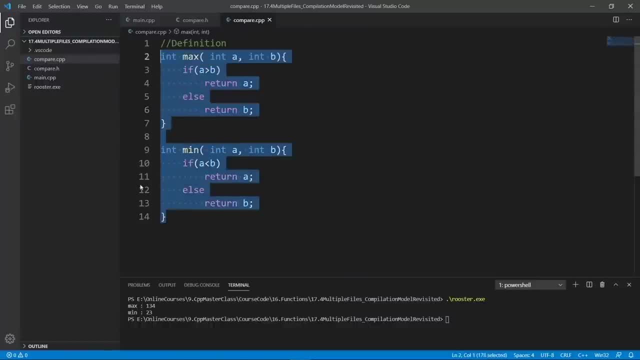 you that we can move this definition there and the program is going to keep working. we're going to add another cpp file and call it some other file that cpp. it has to be a cpp file because it's going to contain the implementations. and let's take the implementations. for example, let's take 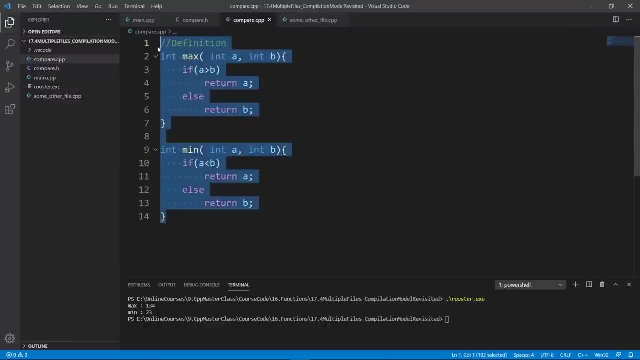 them all and put them in another file. why not? we're going to grab all these guys here. let's cut them out and put them in some other file, and we're going to build this and see that it works. it should, because the linker is smart enough to go. 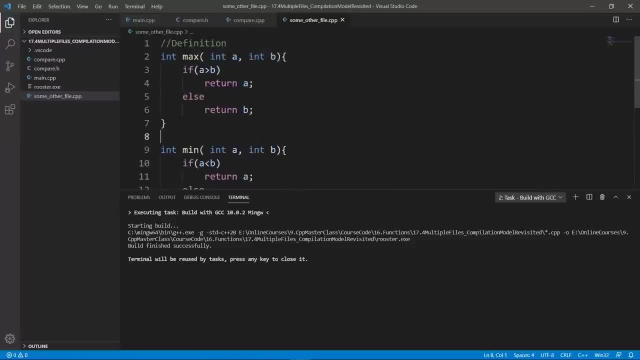 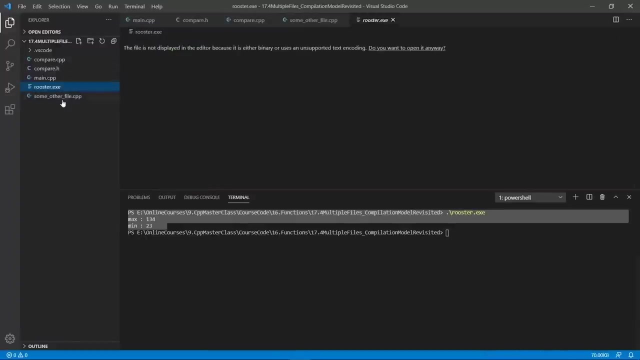 and go find these definitions and whatever translation units that we have set up in our project here, and you see, the world is good. we can build this, we can run this, i should say, and we're going to have our output here. we can even take one of these guys- let it leave- in our comparecpp file, for example. let's take the minimum function here. 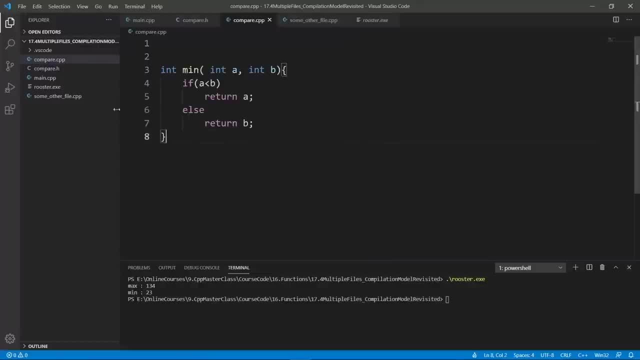 and we're going to bring that back and we're going to world notice that now our maximum function is living in some other file and that the minimum function definition is living in comparecpp. but if we will, this is going to work again. the linker is going to parse all the 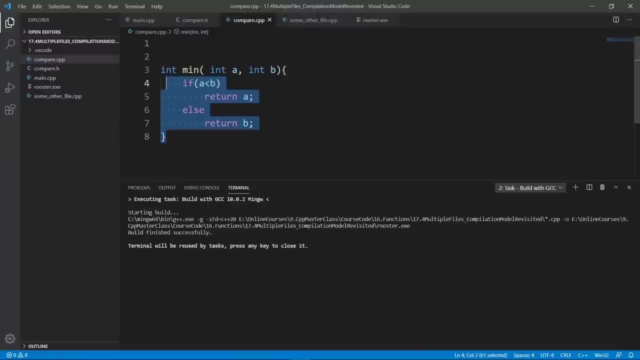 translation units, looking for whatever definition it needs to find, and in this case it will be looking for the maximum here and it's going to find that in some other file, and for the minimum here. it's going to be looking and compare and it is going to find it, and the world is going to be. 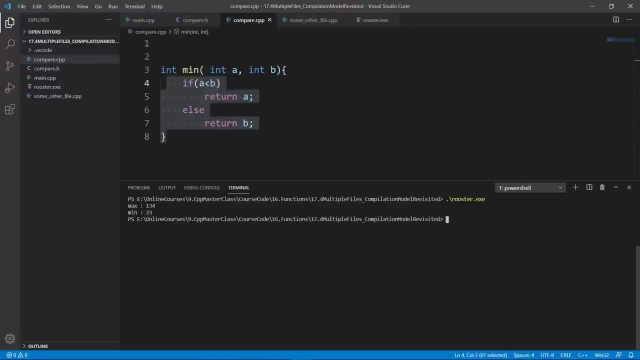 good and we can run the program again and see our output here. one thing i really need to point out is that if the definition is not available- let's say the minimum function here is not there- we can comment it out to hide it to the compiler or hide it from the compiler. and if we try to build now, 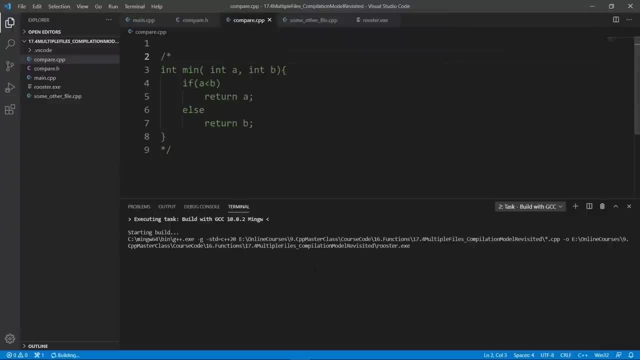 we will get a linker error. let's try to build with gcc. uh-huh, world finished with errors. the terminal process terminated with exit code minus one, but the main message here is that we have an undefined reference to mean and end, so when we compile, the compiler is going to be happy. 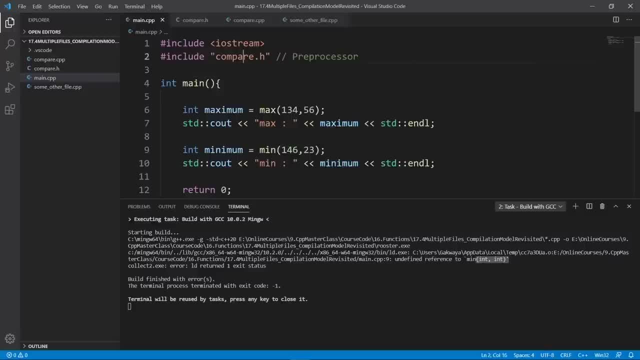 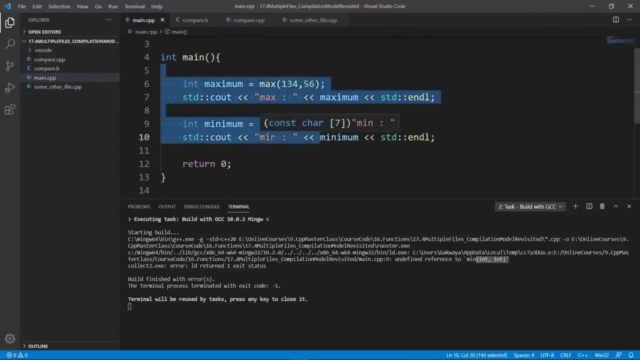 with the declarations that it has found in our compareh file. if we go there, we see that we have a declaration for max and the declaration for man. the compiler is going to be happy, it's going to compile our code. and when the compiler compiles it's going to generate object files and it will. 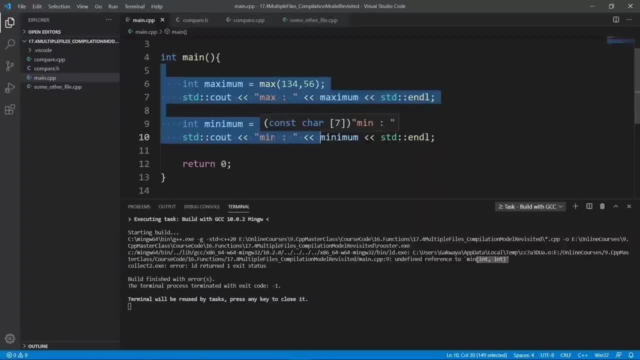 hand the job over to the linker to stitch all those little object files together to have one single binary file. once the linker tries to do that, it's going to look at main, because that's where it's mostly going to start from, and it's going to see: uh-huh, main is calling minimum here. 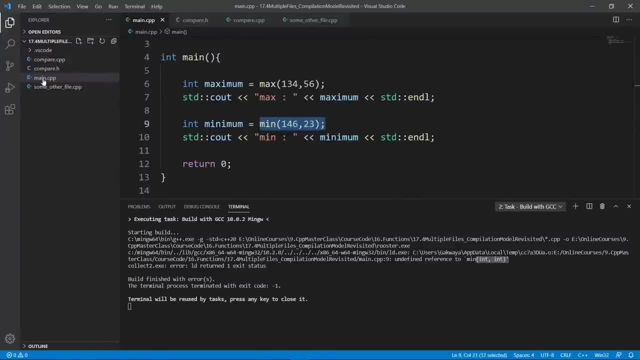 definition for the minimum function. it's going to parse every single translation unit in the project. it's going to come here and compare that cpp. it's not going to find it. it's going to look in maincpp. it's not going to find it. it's going to look in some other file. it's not going to find. 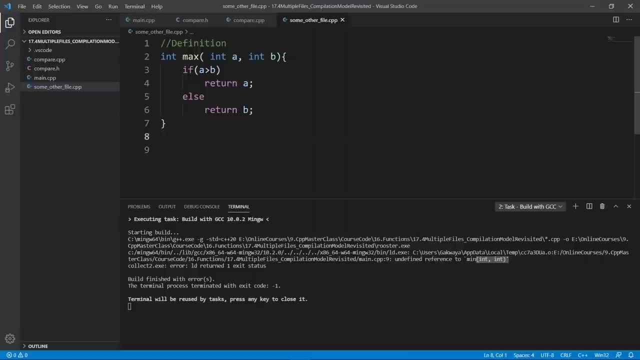 the definition and the linker is going to say: i didn't find my definition for the minimum function, so i'm going to throw a linker error and you, the developer, you're going to fix this problem and you're going to see this error here and again. this is a linker. 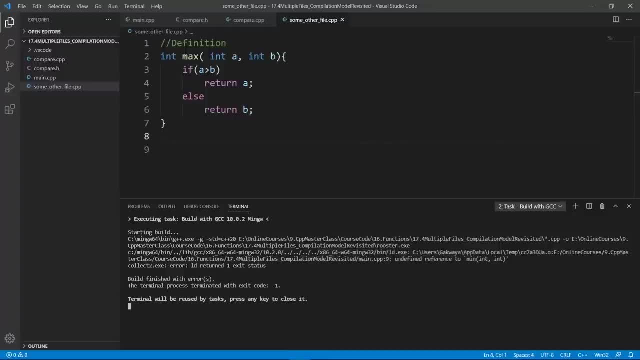 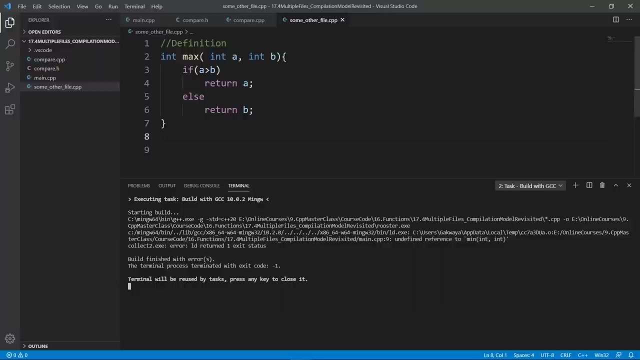 error. gcc doesn't give you more visible stuff to show you that this is a linker error. but what you should look for is ld returned one here, because ld is the linker that gcc uses, so this is a linker error. i think i should show you how a linker error looks if you are using a. 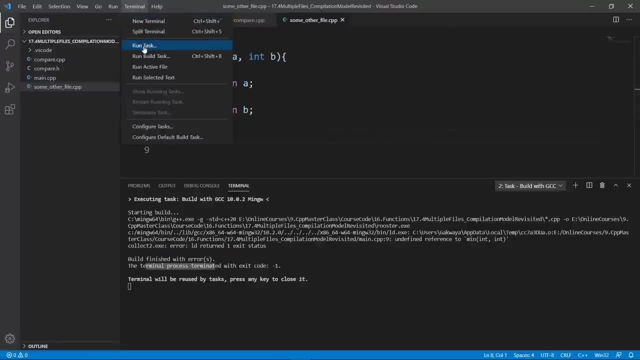 microsoft compiler, so we're going to build again, but now we're going to build with msvc. if you don't, that's not the problem. you can keep using gcc, but i just want you to see how different compilers handle these arrows. i have the luxury to do that because i am developing this course on. 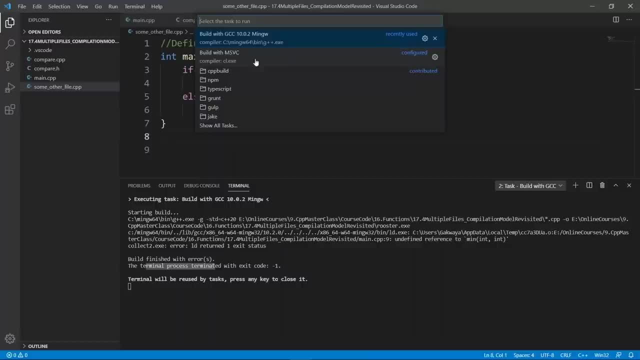 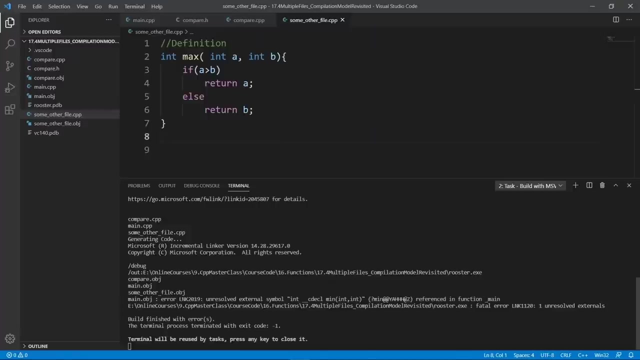 windows machine and i have a microsoft compiler handy that we can use directly from visual studio code here. so i am going to choose this compiler and you're going to see that it is going to start welding. it is welding and it is going to fail and throw a linker error also. so you see here. 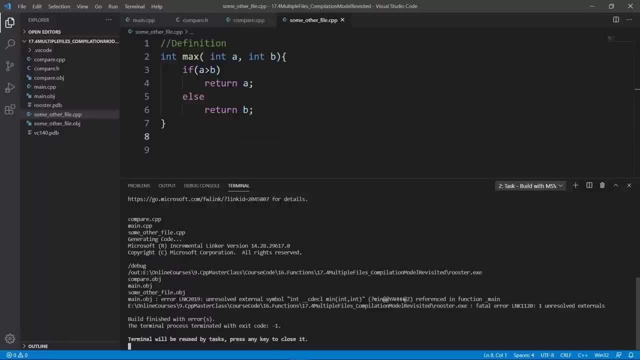 some other object file. okay, when this object file was being taken and stitched together with other object files to put together our binary, it didn't find the definition for the minimum function and it is going to throw a linker error and in visual studio you're going to have a problem like this l. 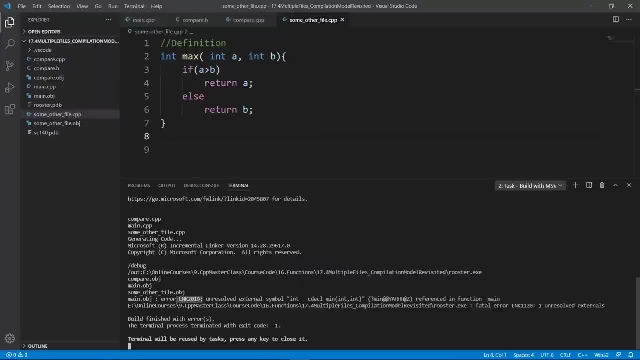 and k and it's going to give whatever version of the compiler you are using. but down here you see unresolved external symbol. this is how visual studio says it and uh, it's basically going to be an undefined reference to something. this is just visual studios compiler's way to say this. 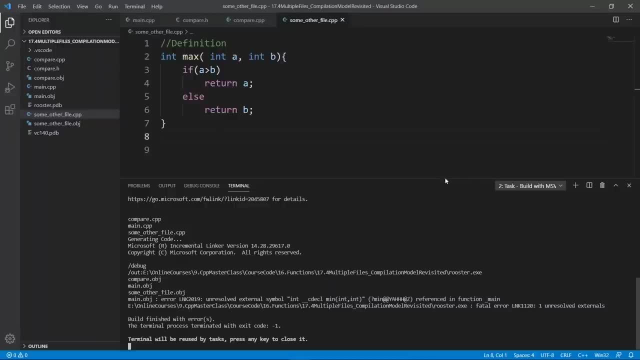 and again it's going to say: this is a linker error here. it is basically the same error we saw when we were using gcc in a minute video studio. the compiler from microsoft is also going to put a lot of junk in our folder here, so let's remove all these things. i'm going to select them all. 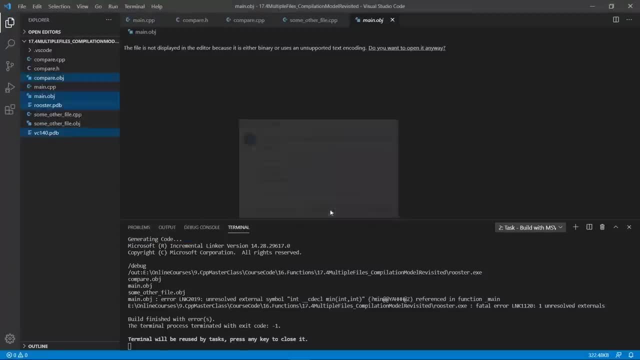 a hit delete here and they are going to go to my recycle bin and we have another one here we should remove. let's remove it. and now we should go back in some other filecpp or comparecpp. that's where we have our minimum function. we can activate it and if we build now, the build should. 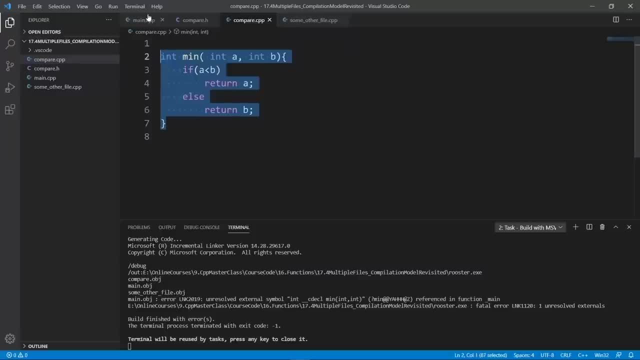 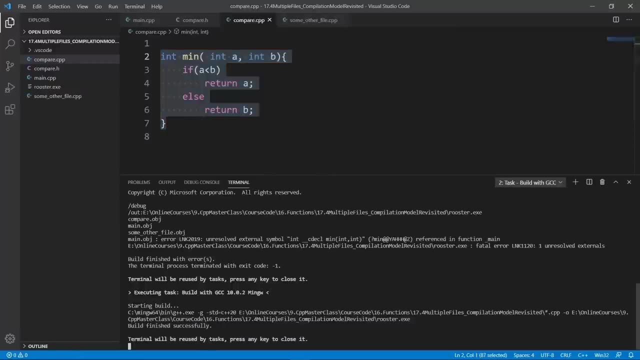 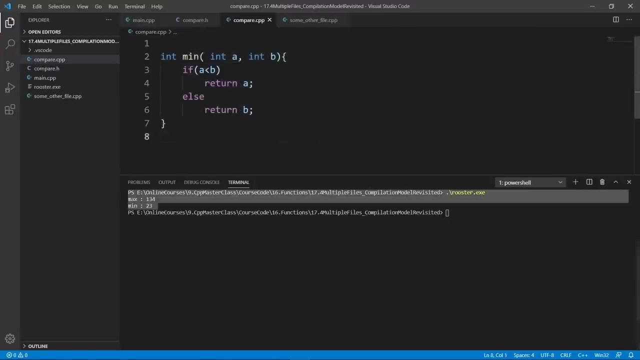 be good, because the linker is going to find this definition here. okay, let's build with gcc, because that's my favorite compiler. now you see that the build is good, we can clear and run rooster and our program is going to work as it should. this is really how you can split your functions across. 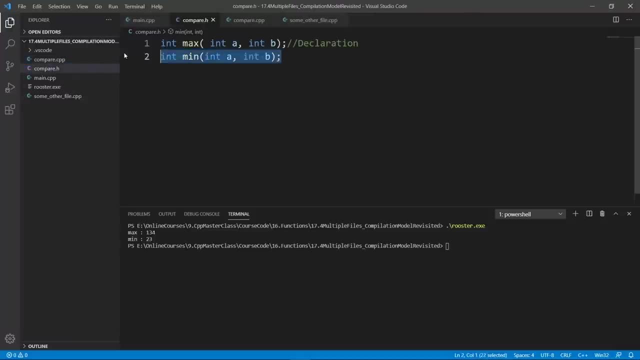 multiple files. the headers are going to contain the declarations. the cpp files are going to contain the definitions. your definitions can really live anywhere. it's going to be a matter of what works better for your project, but for organizations, particularly for the cpp files, it's going to be a matter of what works better for your project. 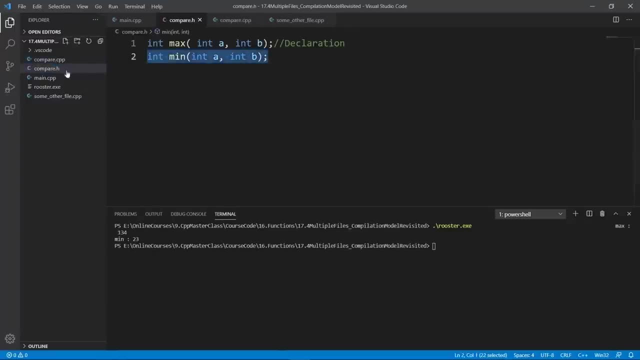 purposes. your cpp files are going to be basically like this: you're going to have some declarations in the header, like compareh, and in a corresponding cpp file you're going to have in the definitions for whatever declarations you have in the header. but you don't have to do it this way if it makes. 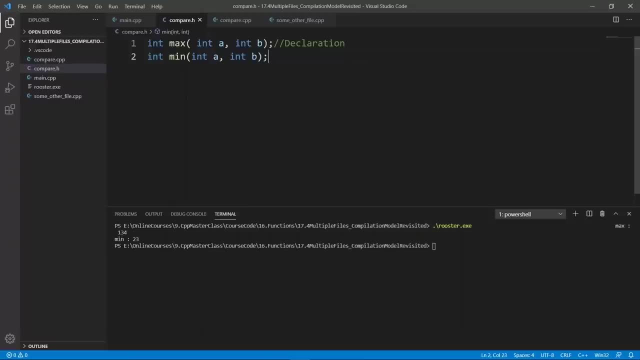 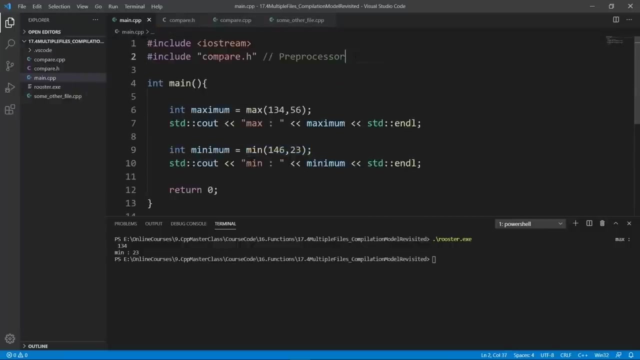 sense for your definition to show up somewhere else. please go ahead and do that. c++ is going to accept that. this is really all we set out to do in this lecture. but before we go, i'm going to give you a chance to set up another function. suppose we have a function called anchor mult and 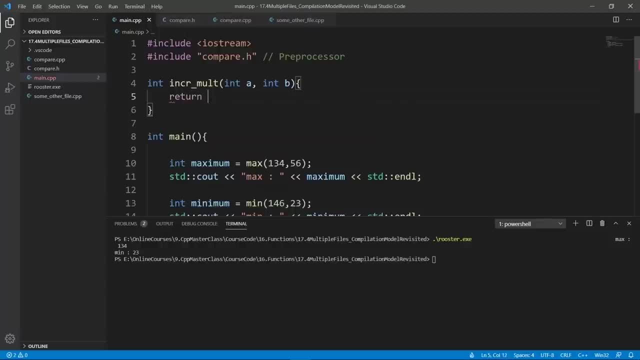 we're going to have the function set up in here. we're going to return a plus plus. we already know how to do this. thanks, we've used this example a couple of times by now. plus plus b, and that's what we're going to return. now your job is to split this function into a deterministic array, and we're 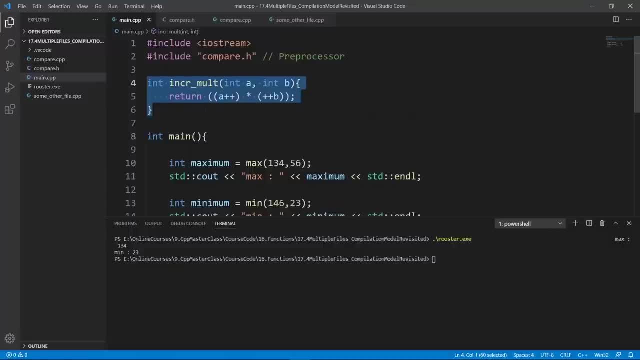 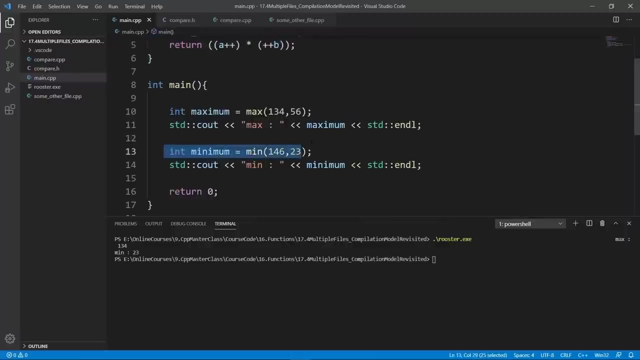 operation and the definition and put those in two separate files. one is going to be called operationsh and the other is going to be called operationscpp. post the video. go ahead, set up your project like that and call that function in main cpp and see if you can pull that together okay. 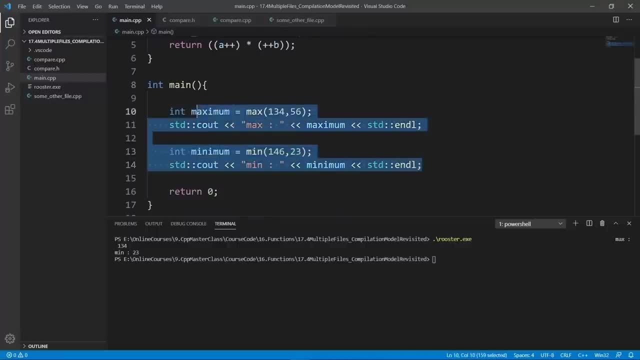 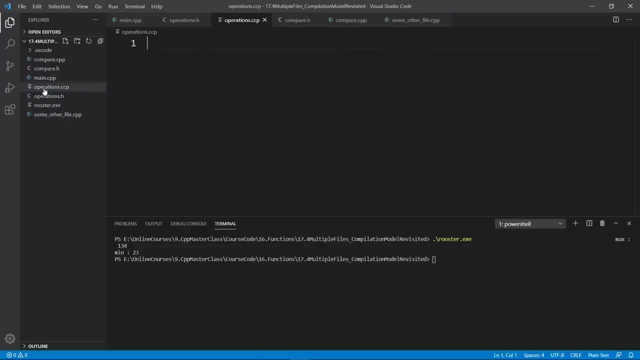 post the video, do that and once you are done, come back again and see how i do this. so we're going to set up a new file called operations here. it's going to be a header file, that h- and we're going to add another file called operationscpp. that's going to be our cpp file, which is going to contain: 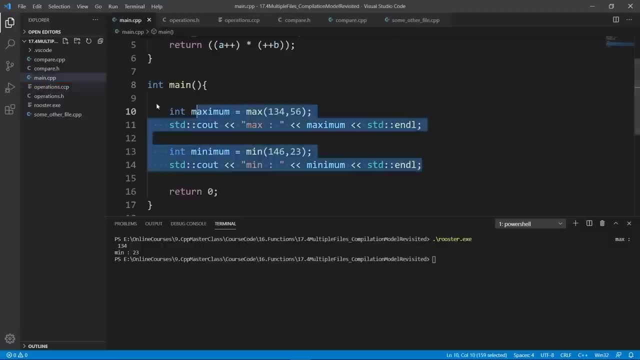 our definitions. we're going to go back in main and grab the entire function here. we don't want it in main, so we're going to go in the header here. we should go in the operations header. that's where we want this and we're going to put in our definition and we're going to put in our. 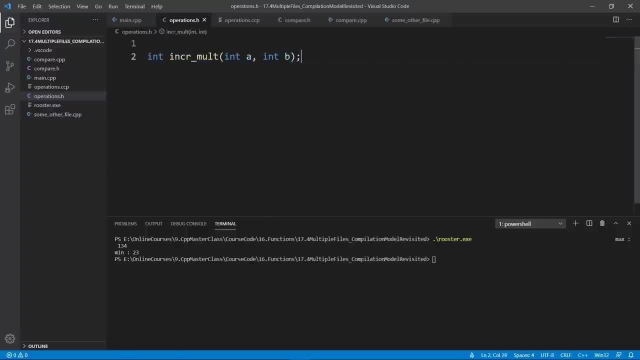 declaration. the declaration doesn't have a body, so we're just going to put a semicolon at the end here. you already know this. we're going to go in the cpp file and put in our definition. this is going to work, and to be able to use this function we will need to include the corresponding header. 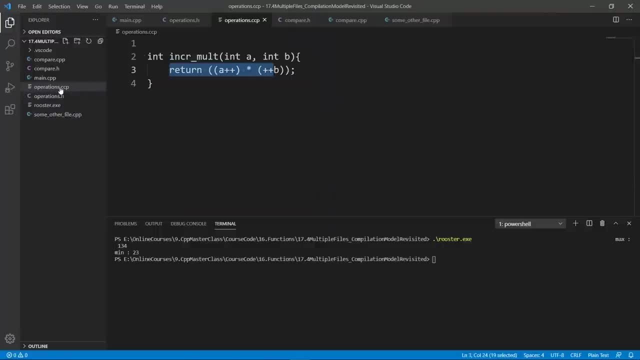 here. why is this file called? oh, it's called ccp. it's cpp. we're going to put in our definition and we're going to go in the operations header and put in our rename it and we're going to change this to cpp. okay, now we should be fine. we should have our 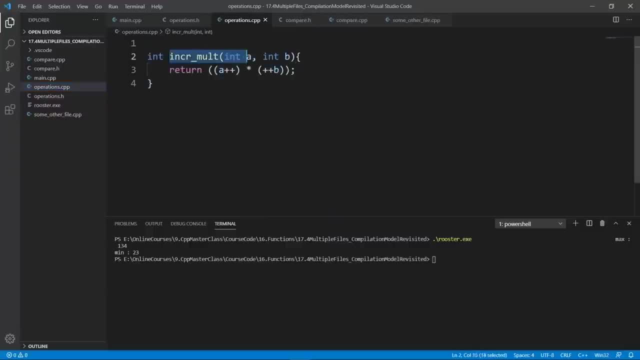 thanks, colored properly and uh, to use this function, we will need to include the corresponding header, which is operationsh. let's do that. we're going to go in main and go down and include operationsh. this is going to work, and notice that the way we include our own headers is different. 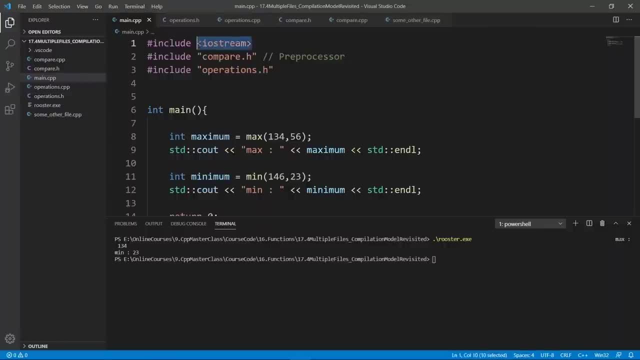 from the way we include the libraries or headers that come with the c++ standard library. this is a conversion that is used by many compilers. this is how we will have to do things. please remember this: if you are including your own header, please put the c++ header in the center of the header. 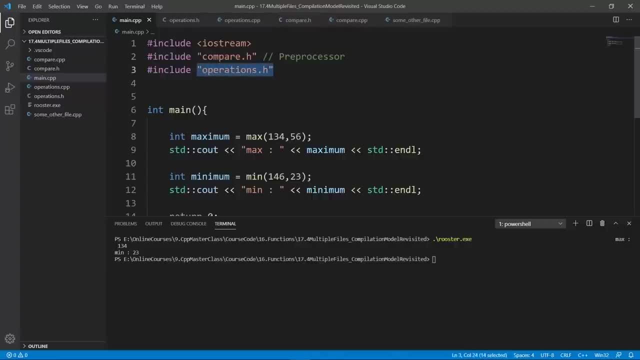 please put the c++ header in the center of the header. please put the c++ header in the center of the header. that in the quotes, like we do here, if you are including a standard library header, please use angle brackets like this. now that we have this included, we can go down here and say result. 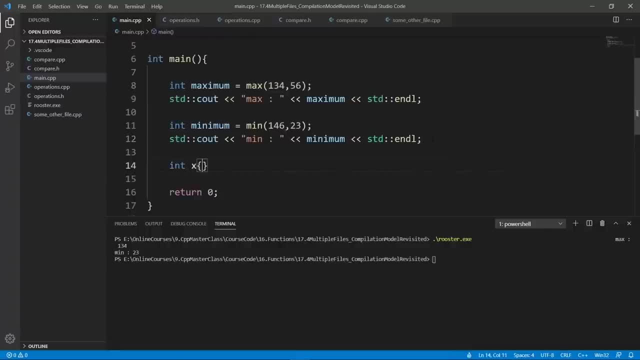 we're going to set up two variables, x and y. why not? we're going to have a four here and we're going to have a y, which is a five, let's do that. and we're going to have an integer to store our result. it's going to say anchor malt. 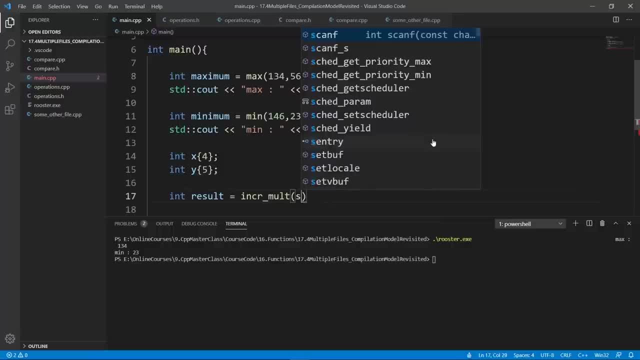 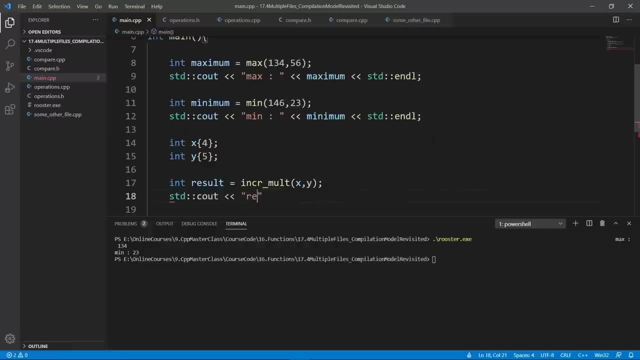 and it's going to do the operations on x and y. let's do that and we're going to print the results here. so we're going to say result and it's going to be whatever we have in that variable. okay, if we build this program, it is going to work. we're going to use gcc to build. the build is good. 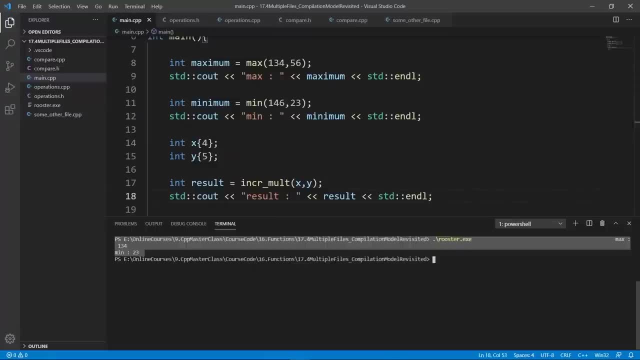 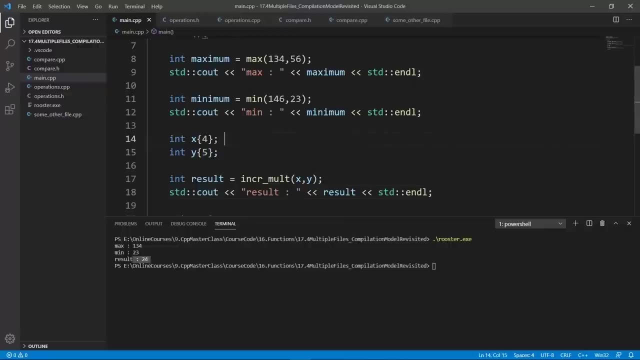 if we run it, we should see our output here. we're going to run root and we're going to run the output here. we're going to run the output here. we're going to run booster and the result is 24 because, okay, if we increment x, we're going to get a five. 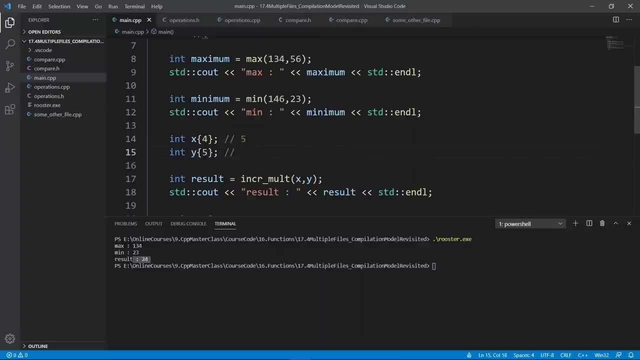 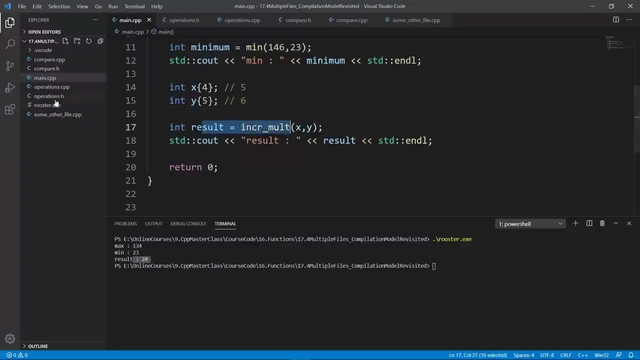 and if we increment a five, we're going to get a six. if we multiply these guys, we should get a 30, and that's not what we have here. so what is happening? let's look at our definition here. ah, we said a plus plus. hmm, we should say plus plus a, because we want to increment immediately. 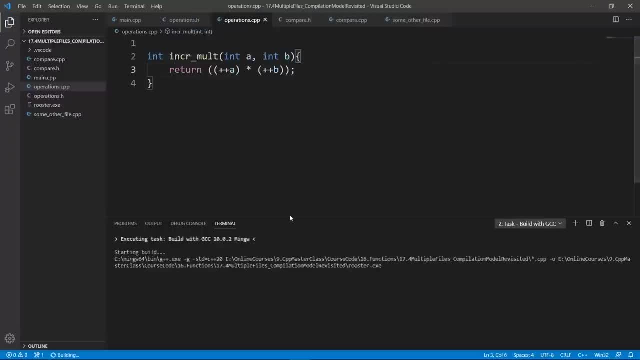 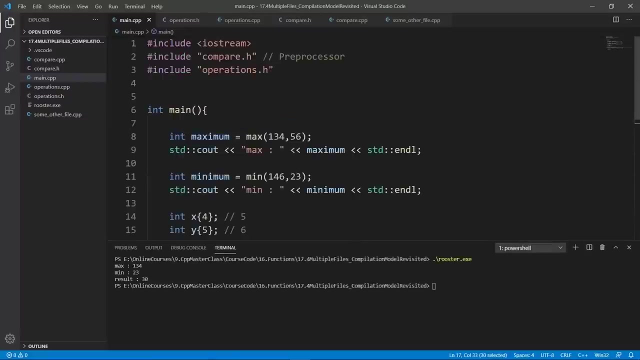 okay, let's build again. we are going to build successfully and we are going to clear and run roaster. now we have the result that we expect. let's go back in main and look at our program. this is what we are using here and this is the output we expect. this is really all we set out to do in this lecture: showing you how you can. 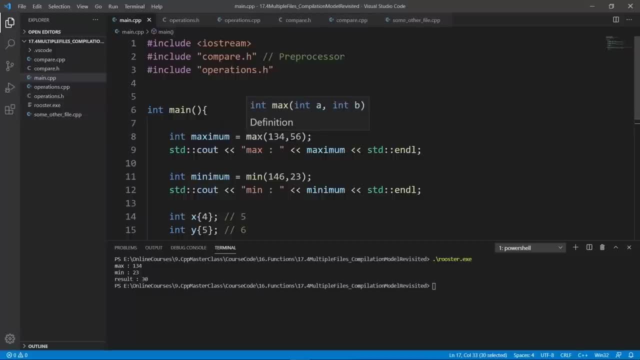 set up your project to split functions across multiple files. this is really good if you want to organize your project. for example, somebody who comes to the header here is not going to be bothered by looking at all the definitions and the details of how we compute this maximum and minimum, and we have the flexibility now to move our headers in some other. 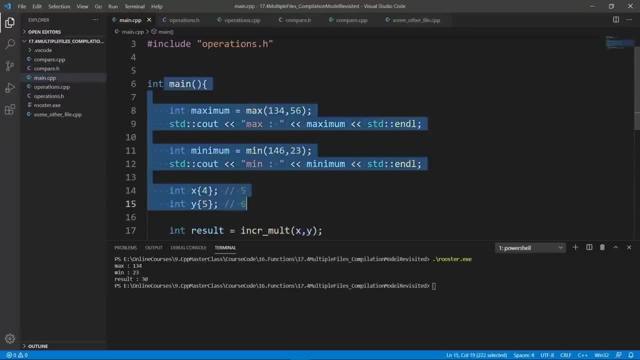 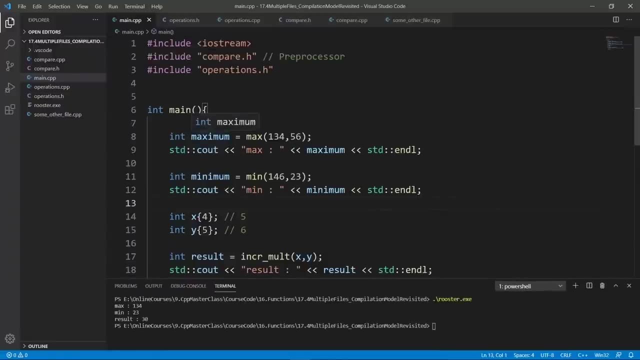 file because we really want to keep the main function or the main file here really clean. we don't want all those definitions to show up here, because it is possible for your project to contain hundreds or even thousands of definitions if you make all those declarations show up. 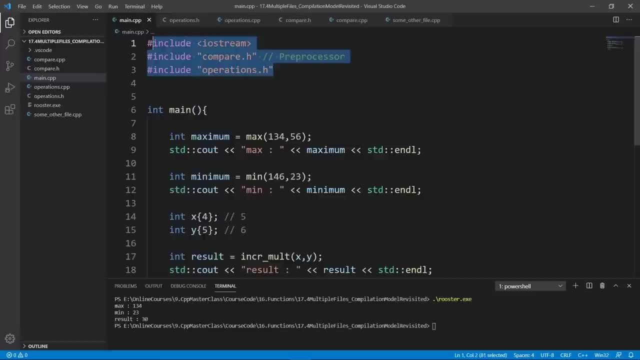 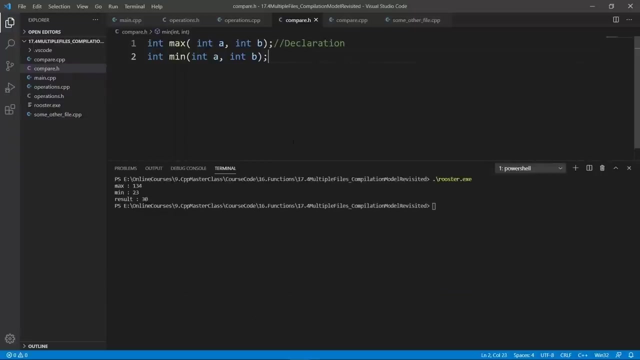 in the main cpp file here. that's going to be really hard to follow and work with. now we have the flexibility to split those guys across multiple files and we can even use lots of headers. if that is what is going to work for our project. this is really all we set out to do in this lecture. i hope. 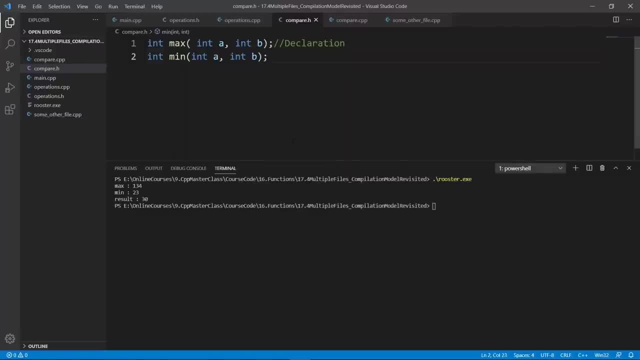 you found it interesting. we are going to stop here in this one. in the next one we're going to see how we can pass parameters to functions by value. go ahead and finish up here and meet me there. in this lecture, we're going to see what is meant by passing parameters to a 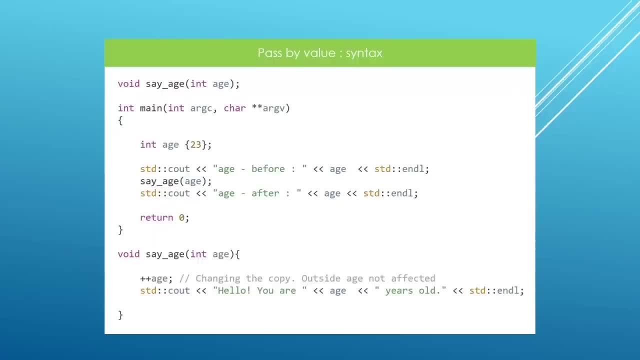 function by value, and we're going to look at an example of that here. we have a simple function called say age. it's going to take one parameter, which is an integer called age, and in the body of the function we are printing out the age after incrementing it. suppose this is something useful. 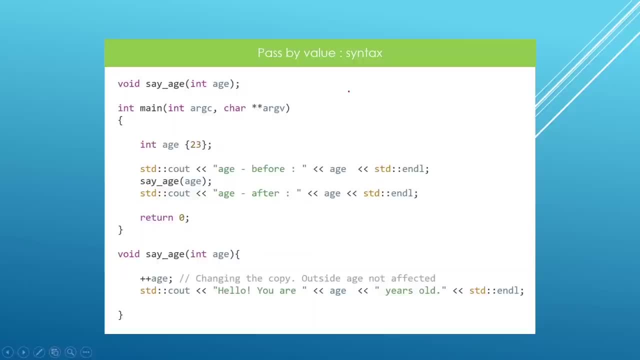 for your program. the function is split into declaration and definition. we have a declaration up here and we have our definition below the main function. in the main function we will attempt to use this function. we're going to call it down here and we're going to pass a local variable. 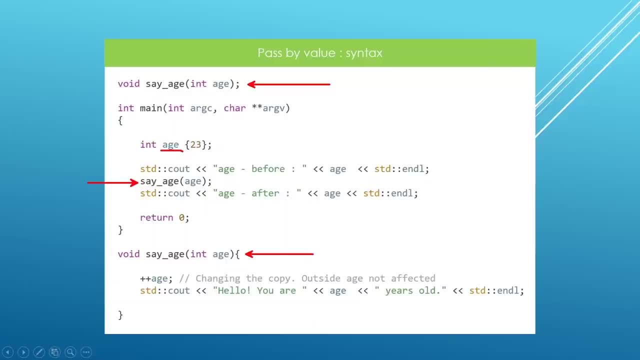 which is called age, as our age. when we do that, we expect this to print: you are 24 years old, because we're going to increment the age and we're going to say: hello, you are 24 years old. this is what this program is going to do, but we want to keep track of how we're going to be able to print this. 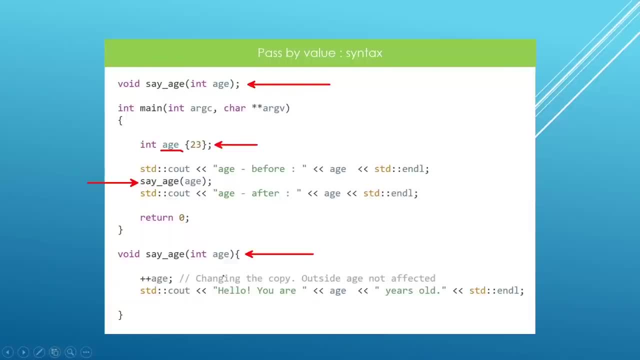 value that is in the에浸 like this, and we want to increase the value so that we get the value when we actually pass the value in the parameter, in the value. uh, that's what we're going to do, is we're going to change the value of the current value here, so we're going to change the value of. 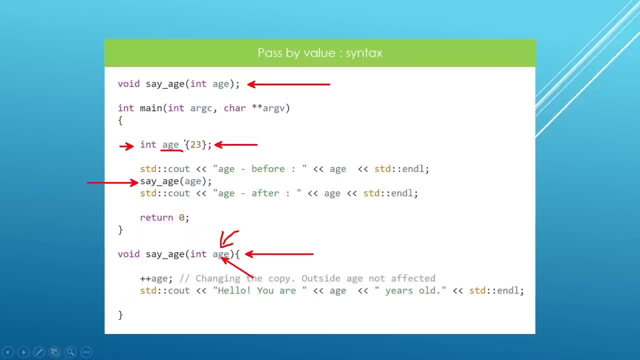 the current value. here you can check and see what are the changes in the learning process. and what's going to happen is that now the outside variable here is going to change and the edge we have passed as a parameter here, because this edge we pass as a parameter. 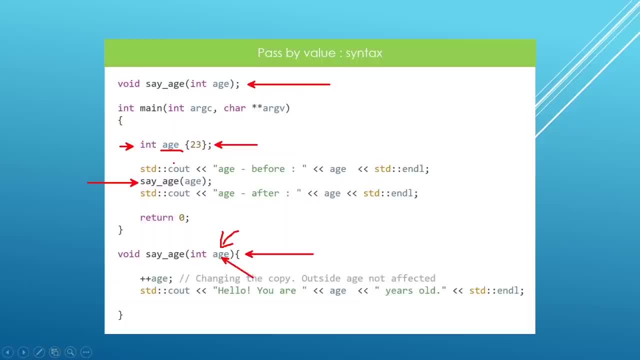 not going to be the original stuff you passed as an argument to the function. so we're going to try and prove that here. we're going to print the age before we call the function, we're going to print the age after we call the function, and what we print here is going to be the outside variable. 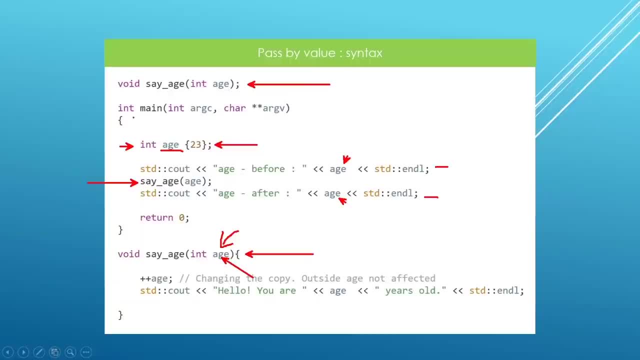 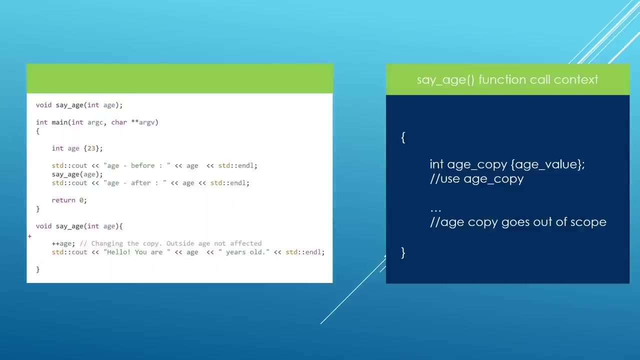 because here we are in the scope of the main function inside the, say, age function. what we're going to be modifying is a local copy, so we expect the age here to stay the same before and after the function call. so the way this is going to work when control has this function here it's like. 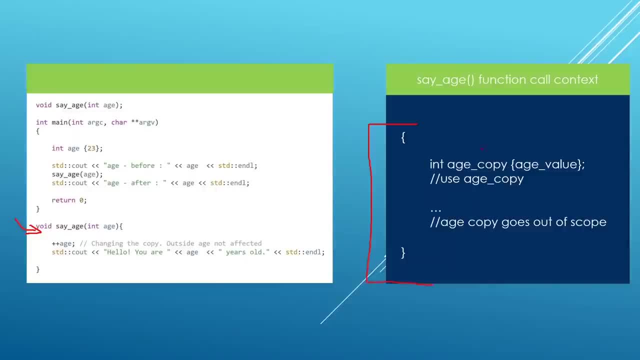 we're going to have a situation like we have here on the left. we're going to set up local copies in the function that are going to contain whatever was passed as an argument to this function, and this age here was passed as an argument to our function, so we're going to have 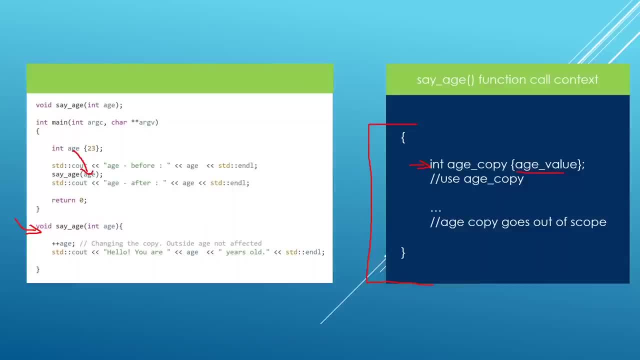 a local copy of this age and we're going to store it, and it is what we're going to be manipulating in our program. when the function goes out of scope, the local copy is going to die and at the outside, the variable we have here is basically going to be unaffected. let's head over to visual studio. 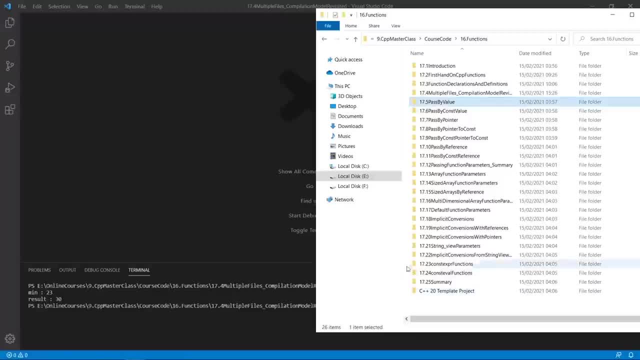 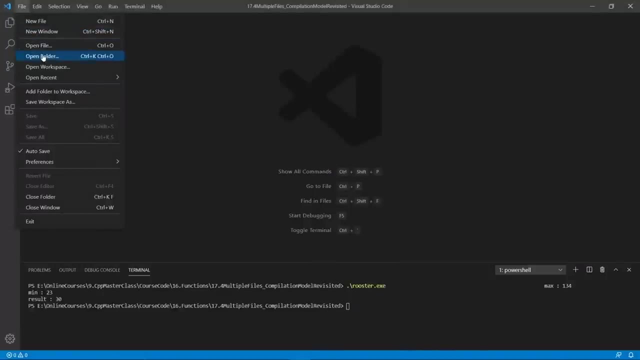 code and show you this in action. okay, here we are in our working folder. the current project is passed by value. we're going to grab our template files and we're going to put them in place in the correct project and we're going to open this up in visual studio code. let's do that, we're going. 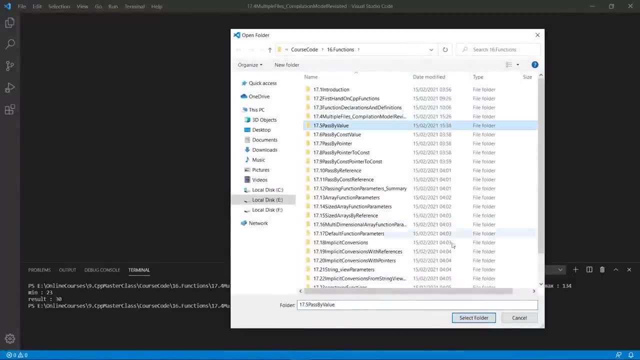 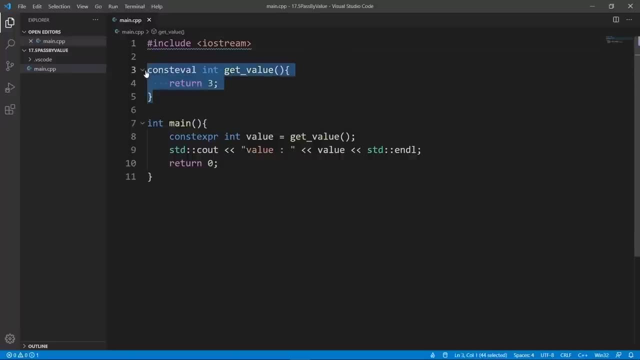 to open the folder that contains the project pass by value. let's do that. we are going to open it up and we're going to go in the file and clean it up a little bit and we are going to set up our function. it's going to not return anything and it's going to say age and it's going to take an. 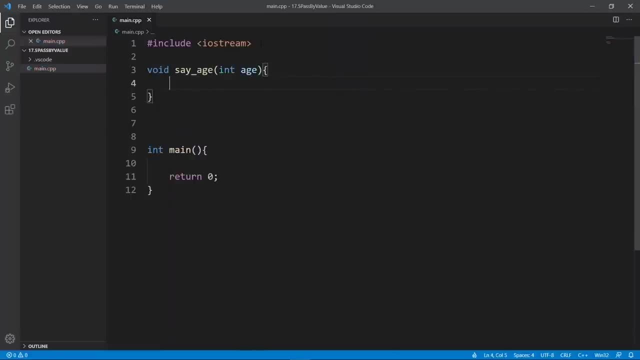 integer, which is going to be our age, and inside we're going to increment our age. i think this is what we saw in the slides and we're going to say: however many years you are old. we're going to say hello, you are age old, and we can set up a variable in the main function. we're going to call it age. 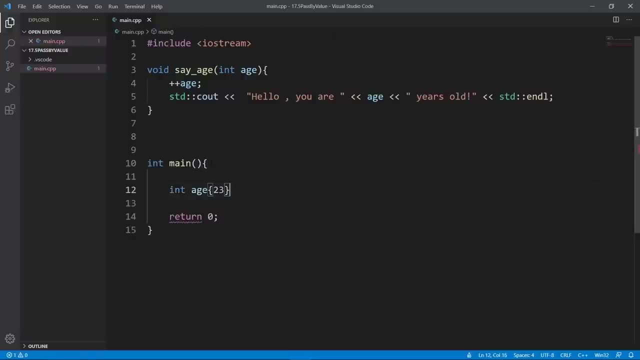 and it is going to contain 23 as our age. we're going to say age and we're going to pass in our age here. we can do that. if we're trying to run this program, let's try to do that. we're going to build with gcc and we are going to bring in a terminal. 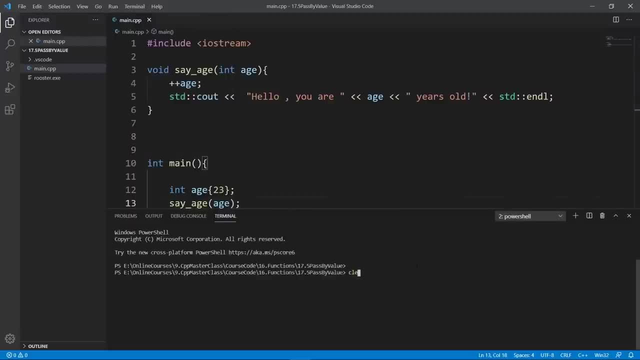 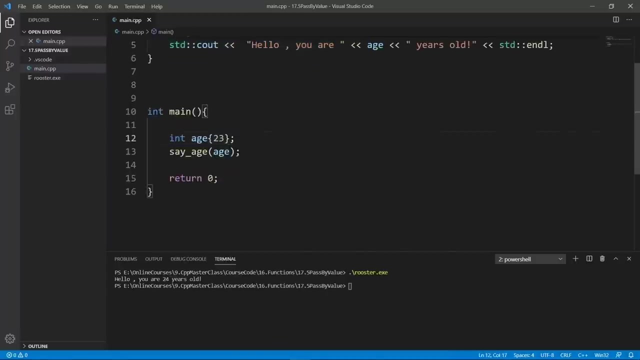 we can use to run this program easily from visual studio code. here let's run booster. we're going to say hello, you are 24 years old. and this is what we expect, because when this function is called, we're going to increment the age. then we're going to say the age, but we want to see what happens to. 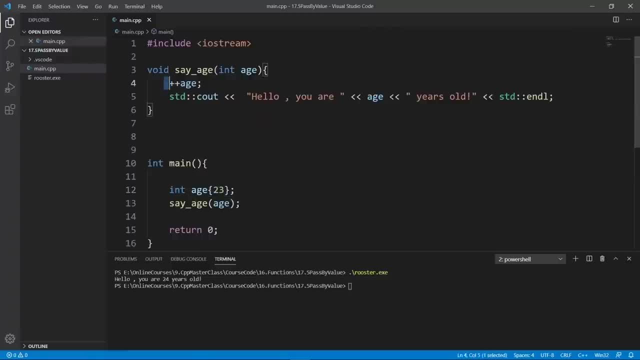 the outside age here. if we modify the inside age that we have on this function here, that was passed as an argument and again, what you pass when you are declaring your function is a parameter and what you pass when you are calling the function is called an argument in. 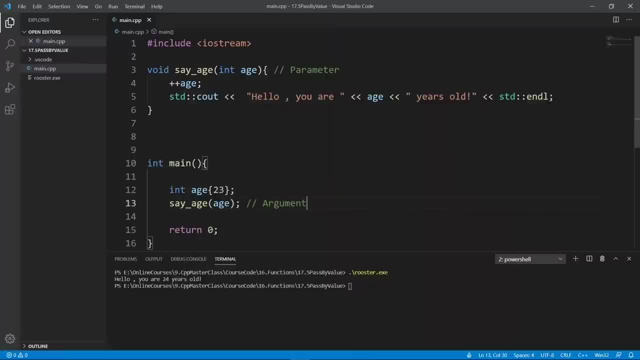 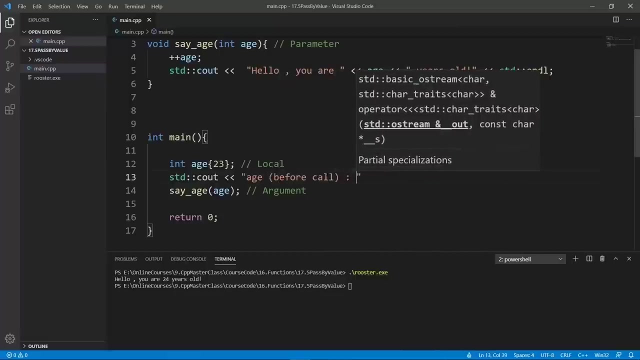 c++. please remember this. okay, what we pass as an argument is our int age variable, which is local to the main function, and we're going to see what happens to it. let's print the age and say age before call. i think this is descriptive enough and we're going to print the age. 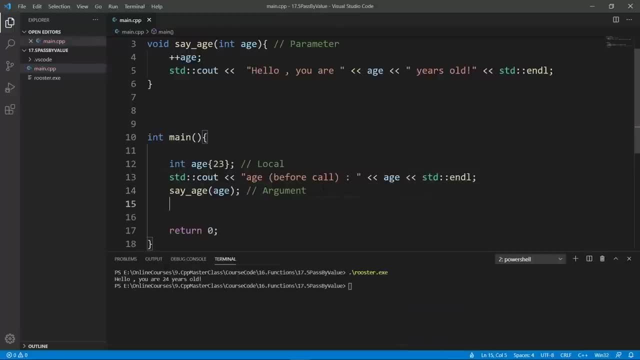 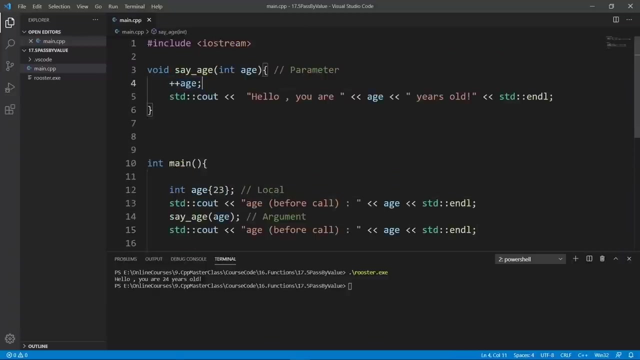 that, and we're going to go after the function is called. we're going to say the same thing, but we're going to say after call, and by after we mean after we call the function, say age. here i think this is descriptive enough and we're going to see that if incrementing the local variable to the 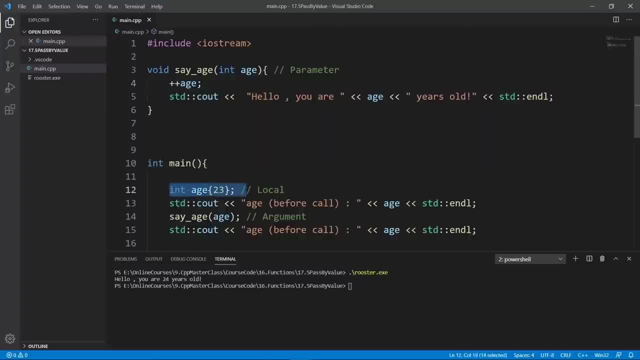 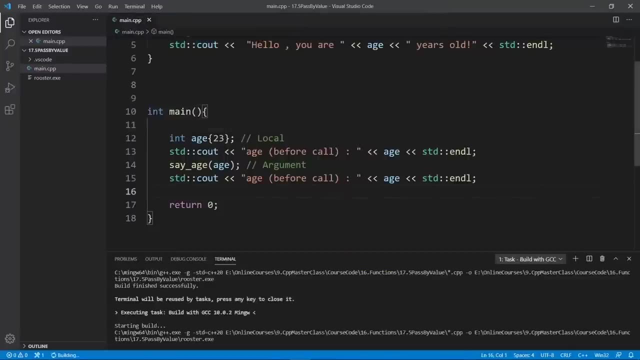 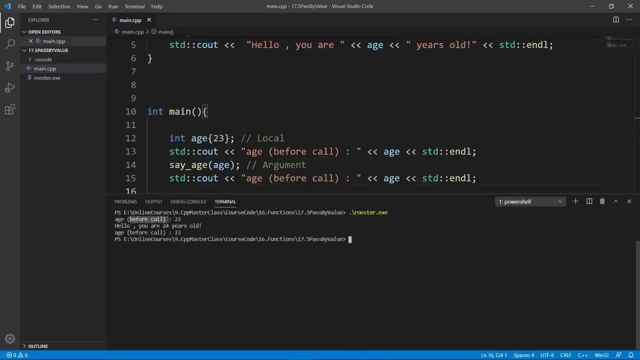 function here affects the variable that we have in the scope of the main function. okay, so let's see that we're going to build with gcc, as always, and the world is good. so let's clear and run rooster. you're going to see that before the call. 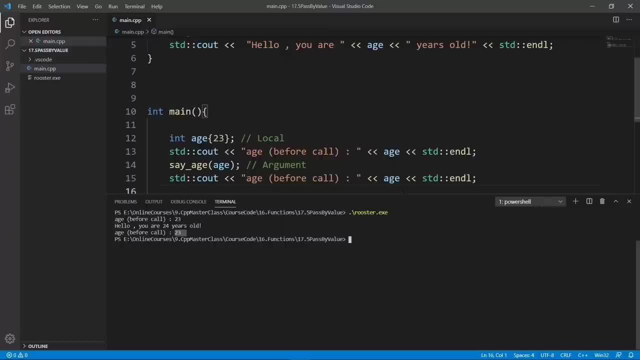 we have 23 and after the call we have 23. we didn't change the second call. this is a classical copy paste error. we're going to change that for our program to really be descriptive enough. okay, the world is good, we can clear and run rooster. and now we have, before call, 23, after call. 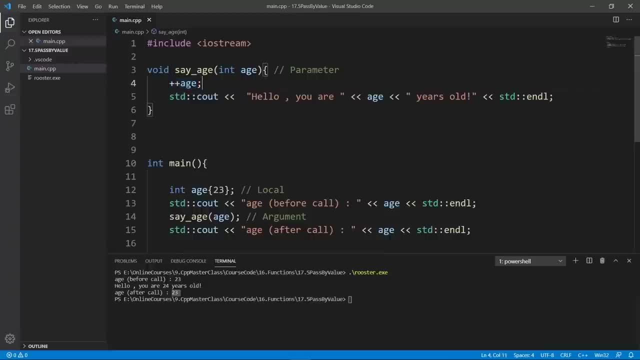 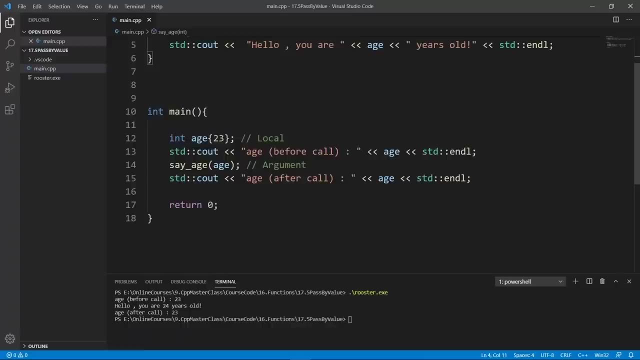 age is 23. it wasn't changed by one of the functions that we have in the program. so we're going to see that. so we're going to go back here and see what we have inside here, and we can even go further and look at the memory addresses of these guys. here we can try and print the address of the age variable. 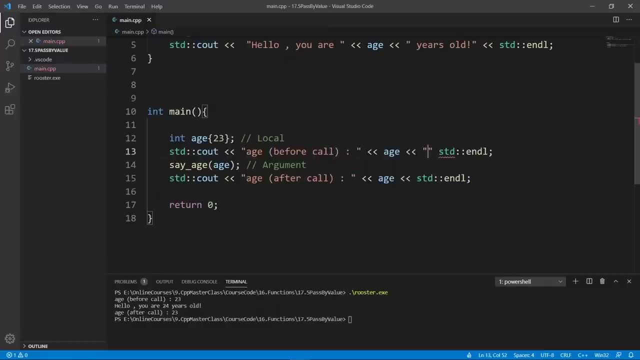 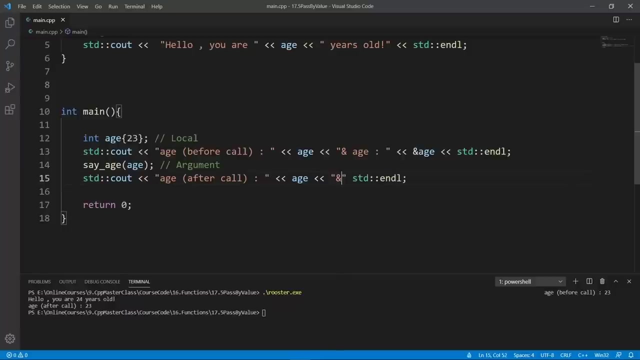 let's do that. we're going to say address of age and put that out here. we're going to say address of age, no big deal here. we can close the pane on the left here because it is taking up valuable space and we're going to go to the second statement. 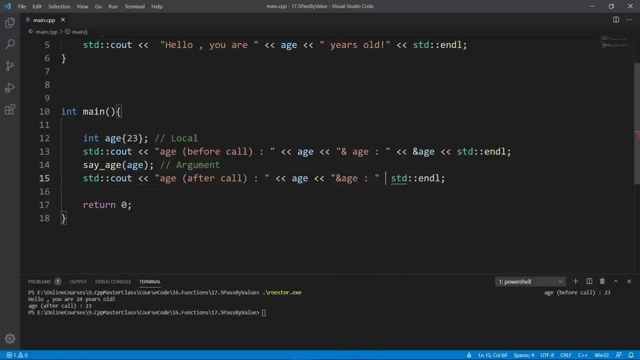 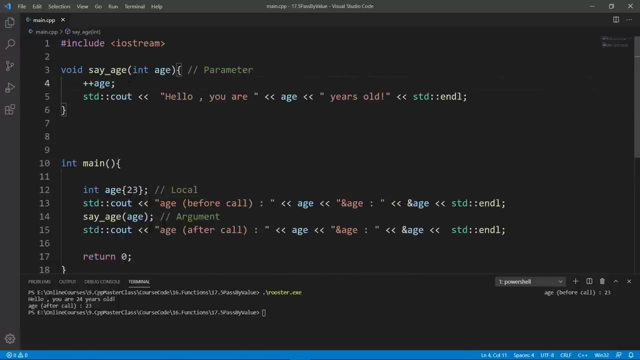 and put in the address of age and we're going to print that out. we can do that. now we know the address of operator. okay, we can do that. and when we hit the body of our function here, we can also print the address of age. no big deal. so we can say: address of age. let's do that here and 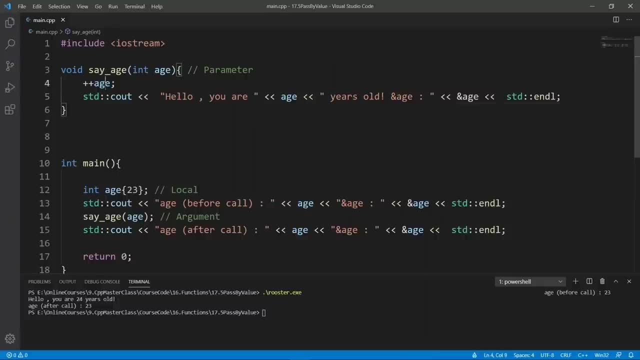 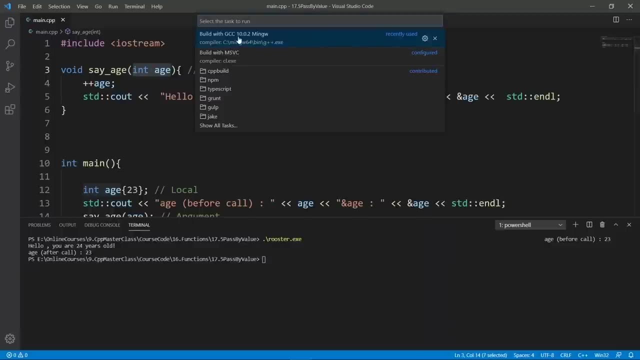 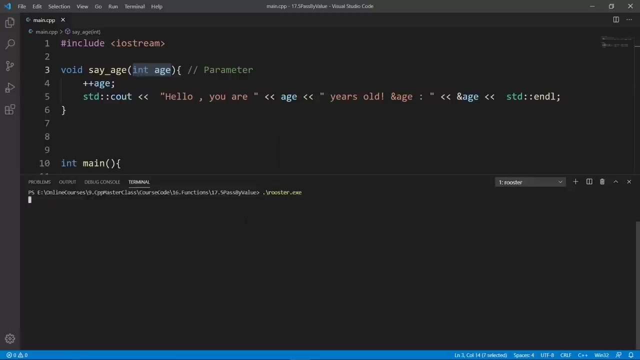 we're going to print the address of the local age variable here, which was passed as a parameter here. okay, now we can build our program and watch those addresses. we're going to build with gcc. the build is good. we can clear and run rooster. now you see that the outside variable is going to. 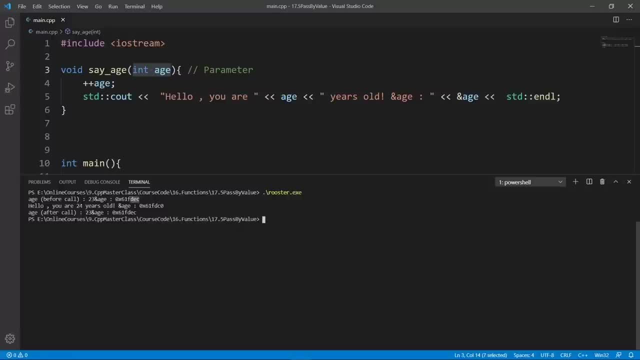 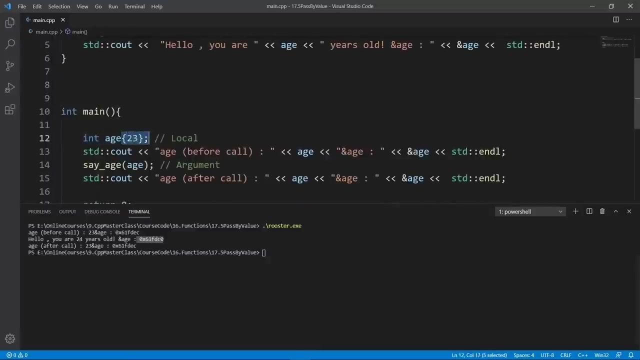 leave at an address that ends in dec and the local variable is going to leave at an address that ends in dc0. so this is a completely new memory location that we are using, and it is just going to contain a copy of what we passed as a parameter here, and the compiler is going to take care of setting up this. 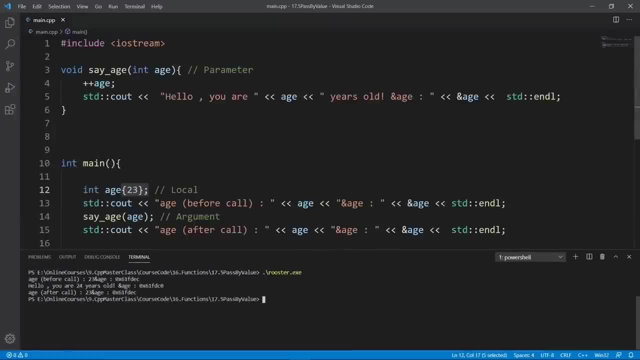 copy variable and have it available for use in the local function. here we don't have to worry about that. but we have to be aware that what we are working on and the say age function here is a copy. it's not the original value. this is really all we set out to do in this lecture. 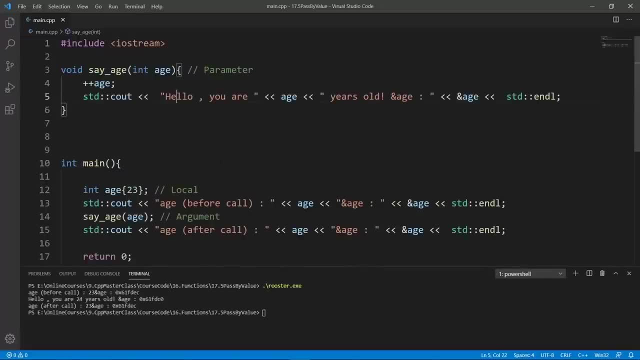 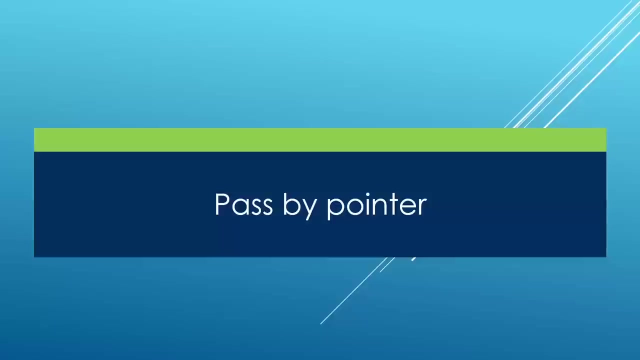 making you aware of the call by value mechanism, and the main message is that what you are working on in the body of your function when it is called is going to be a copy of what you have passed as an argument when your function was called. here in this lecture we're going to see: 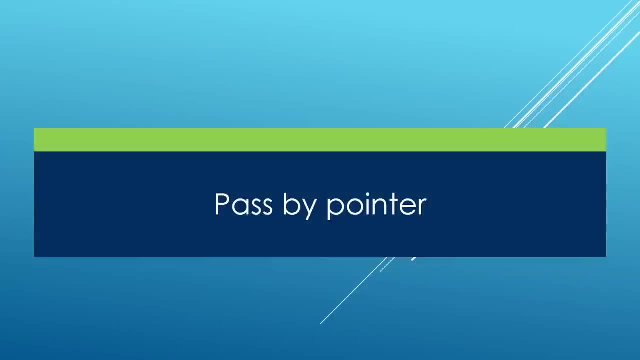 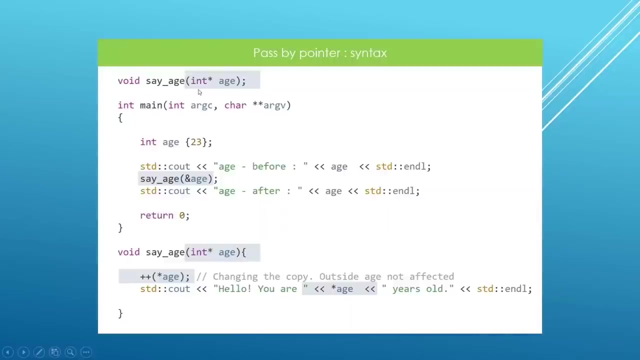 how we can pass parameters to functions by pointer. this is going to allow us to avoid the copies that we were experiencing when we were passing parameters by value, like we have seen in the last few lectures. here is a simple example showing the syntax used to pass parameters by pointer. on top here we have our function declaration and down here we 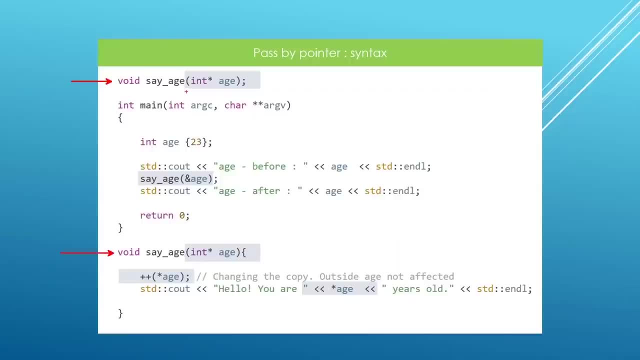 have our function definition and you see that the syntax is the same. we are passing by pointer and by pointer in the definition here, and another thing you should be careful about is that when you call a function that passes by pointer, you have to give it an address, and that's what we are doing. 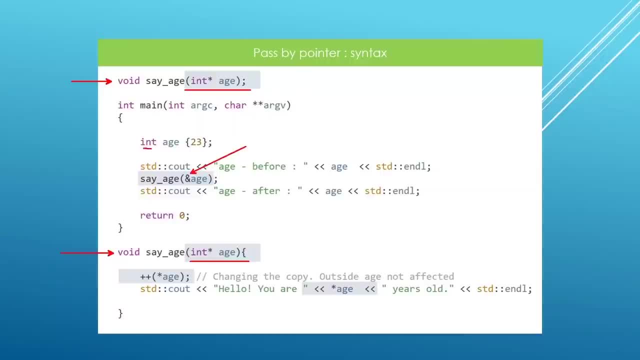 here. so we are passing the address of our age variable which is going to be passed by pointer. when we pass by pointer, we want to be modifying a copy inside the body of our function. if you look here we are incrementing the age variable, but we are doing this through the referencing. so when we 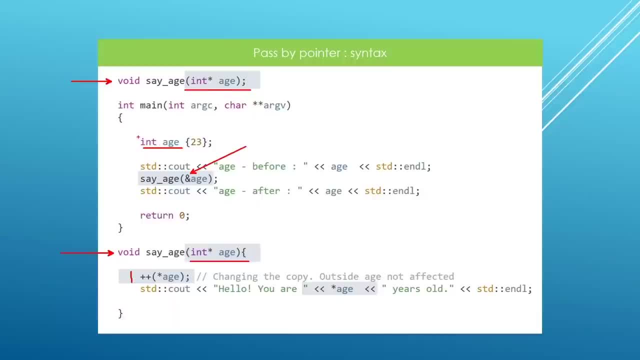 pass a pointer here. the pointer is going to contain the address of this guy and in the body of the function, the point we will have this age pointer is going to be pointing to the original variable here. okay, so this age pointer is going to be pointing to the original age variable when we dereference it. and 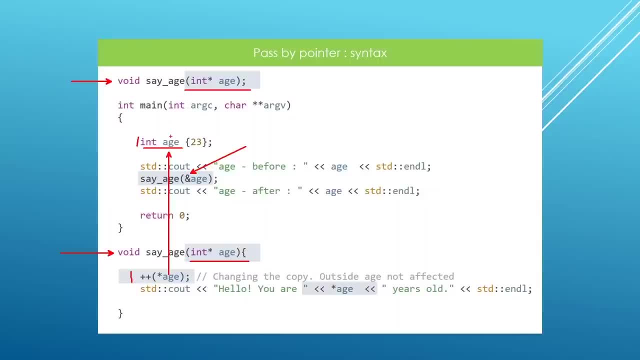 modify the variable, we're going to be affecting the original variable. i really hope this makes sense. and this is really what passing by pointer is all about. you declare your functions by passing in pointers like this, and in the definition you do the same, and when you call the function, you 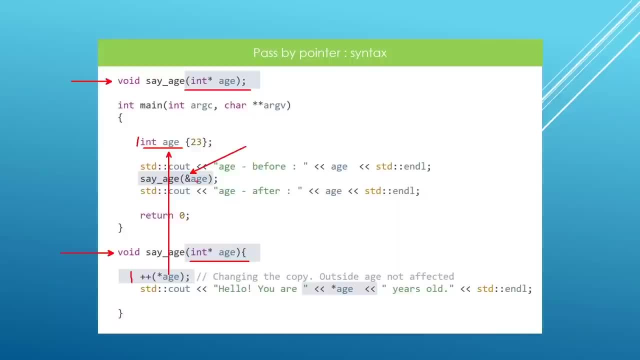 need to pass in an address of the variable, because that's what we store in a pointer here and this is going to work. if we're trying to run this example here, we're going to print 23, because that's the original value. we are going to call this age, we are going to increment, and this is. 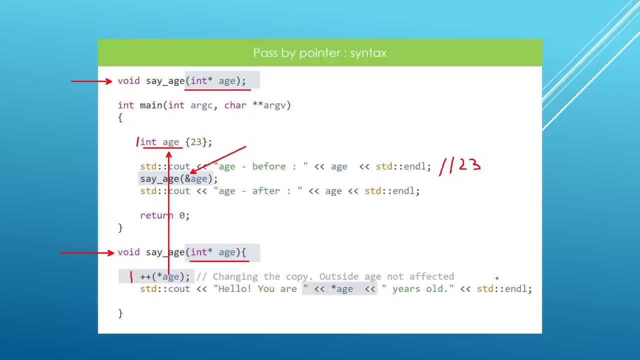 going to change the original value. if we print here, we're going to get 24, and when this function terminates, we're going to hit this statement here and we're going to print 24. this is what we're going to see here, and we're going to print 24.. 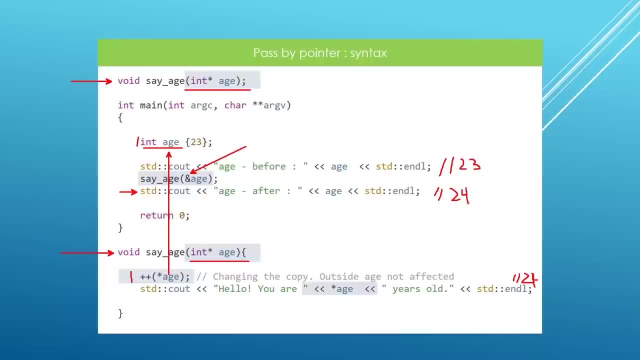 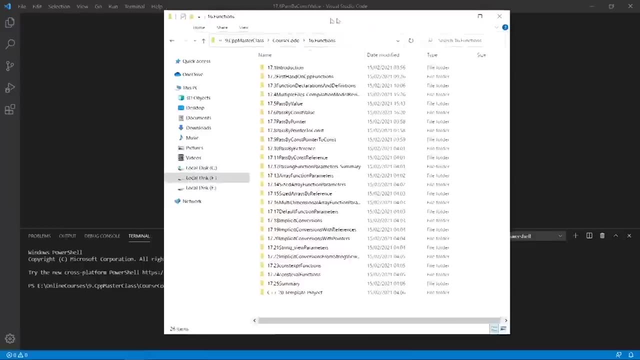 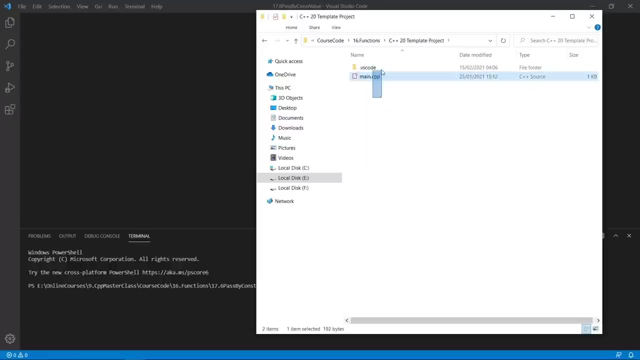 see when we get to run this program here. and this is really all there is about passing by pointer. we are going to head over to visual studio code and play with us a little more. okay, here we are in our working folder. the current project is passed by pointer. we are going to grab our. 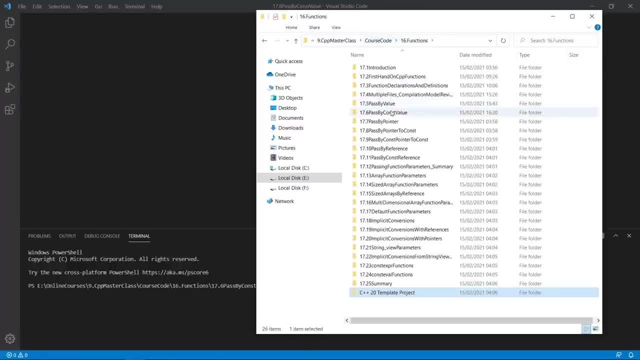 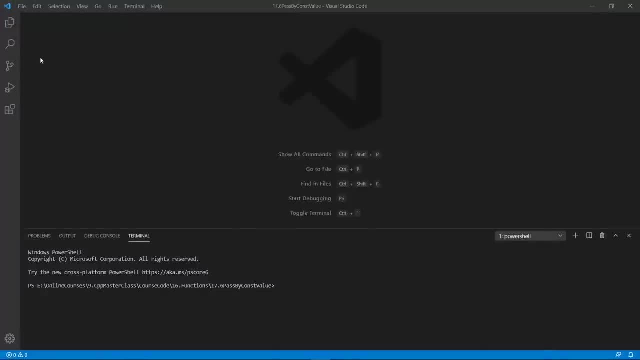 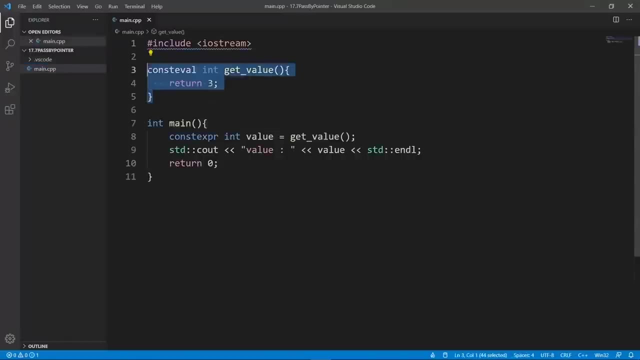 template files here and we're going to put them in the current project, which is passed by pointer. we are going to open this in visual studio code. pretty quick, we're going to choose that pass by pointer. we open this and our main cpp file should show up here. we're going to clean. 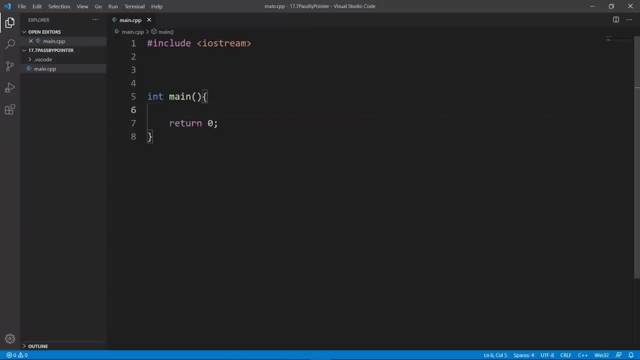 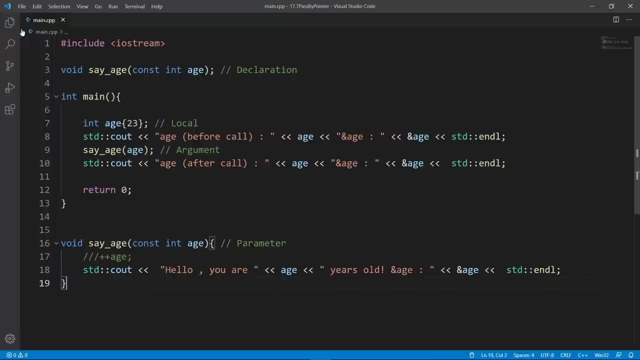 it up a little bit. we are actually going to grab the code from the last lecture and put that in here, and that's going to be our starting point. let's close the left pane here so that we have some breathing space. the function here, say, age, is going to pass by pointer and we're going to 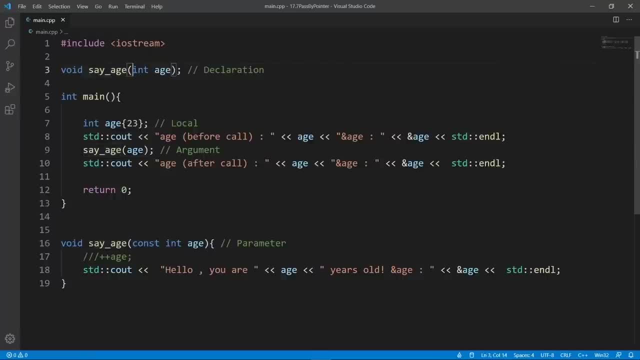 pass it the address of the class that's written here in our new function say age. so that's what we're going to do. let's close that up and we're going to go back in and we're going to do the same in our definition here if we go down. we're going to do that, we're going to pass by. 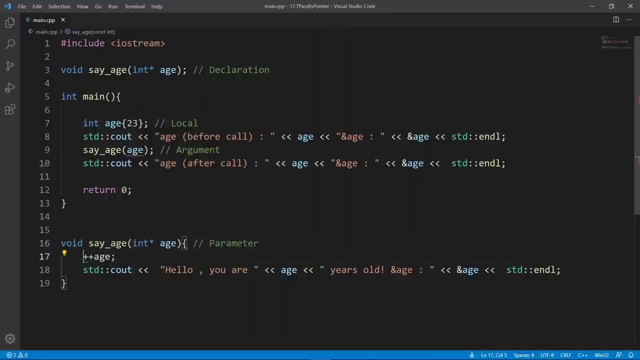 pointer and we are going to uncomment the line that increments our age here. okay, after we do that, you see that we have a squiggly line to this line that calls the say age function. what we need to do is to pass it the address of the class that's written here, and we're going to do that. 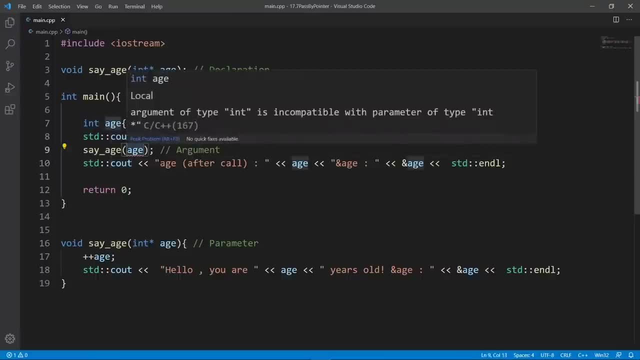 edge variable here, like we saw in the slide. so this is the syntax we have to follow. once we do this, this program is going to be valid and if we run it here, we're going to print 23, because that's the value we have in here. we're going to call this a age function, we are going to increment age and 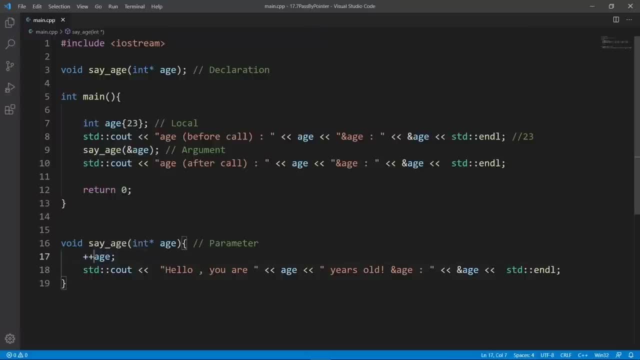 here we forgot to do our dereferencing, so what we need to do here is to dereference the age and increment it. this is going to increment the original variable here and we're going to be accessing this through the dereferencing operator of our pointer here. if we hit this line in the 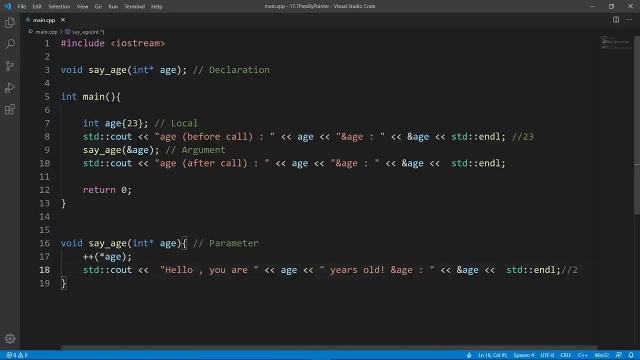 function here we're going to print 24 because the value has been incremented through this statement here and after the function call, we're going to hit this statement here on line 10, and it is going to print 24. this is what we expect. take a moment to make sure you really understand this. the things you need to be careful about. 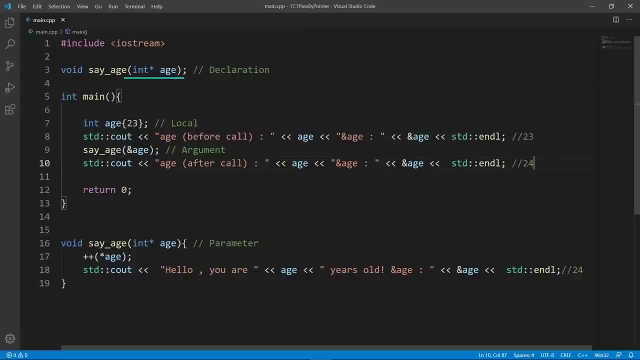 is the syntax we use to declare the function. here we say that we are passing by pointer because of this little star here. and we have the same thing when we hit the definition of the function. we have this little star, so we are passing by pointer. another thing you should remember is to pass. 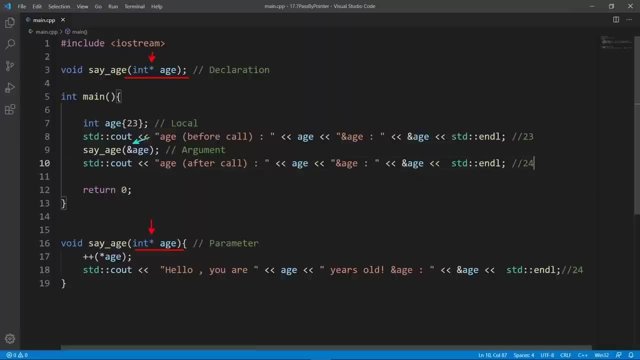 the address of a variable when you call the function, like we do here, and please remember to use the reference operator whenever you want to modify. whatever variable is leaving at the address that you passed in here. so that's why we are dereferencing here through the star operator, like we are doing here. this is really all you need to be careful about. 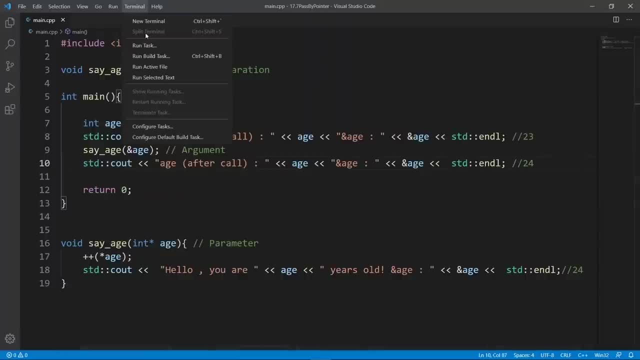 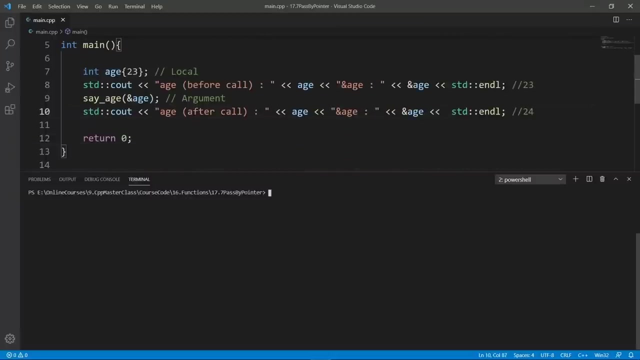 so we are going to try and run this program. let's do that. we're going to build with gcc. the world is going to go through. we need to bring in a terminal so that we can run this program, and we expect to see a 23,, 24, and 24 here printed out. 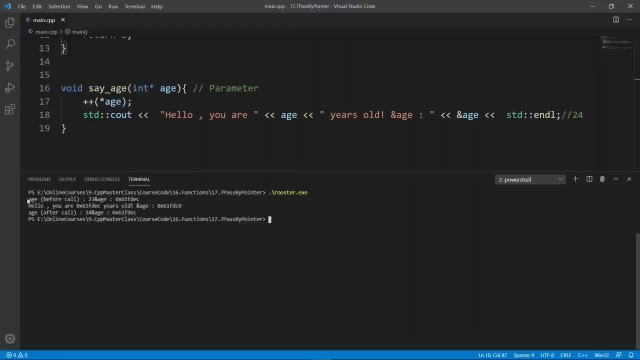 So let's run rooster. Okay, here is our output. before we call the say age function. the age is 23,. the address is DEC. When we hit the function, we are saying: hello, you are years old. So here we should have the referenced. 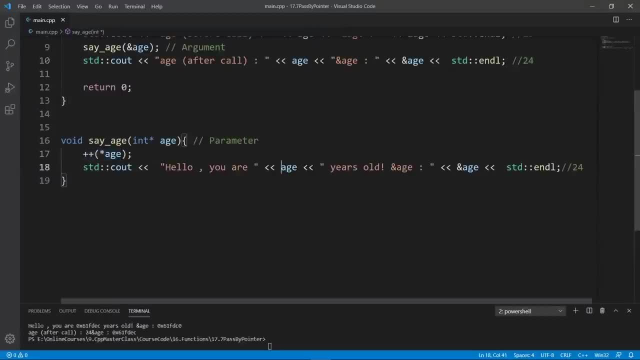 to access something inside the variable here. So we should say: you are age old. We need to reference this guy because now it is a pointer. I forgot that. I really am sorry, but we are learning, So this is a good learning chance for you. 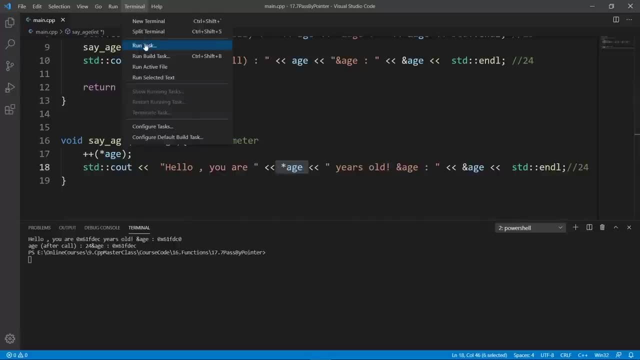 not to make the same mistake as I am making here. So let's try and build again. We should see the correct output. We are going to clear and run rooster. Now we see that before the call, age is 23.. When we call the function, age becomes 24. 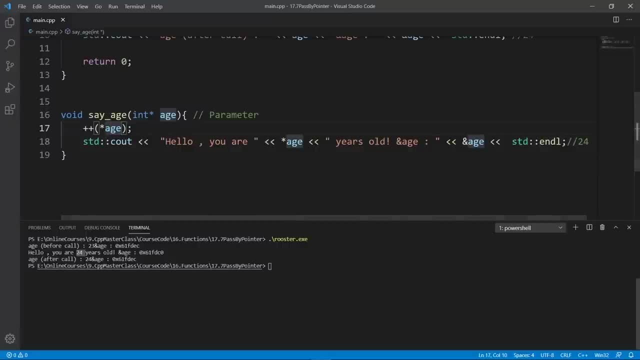 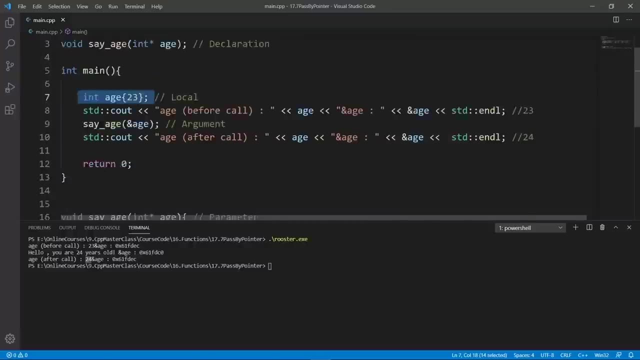 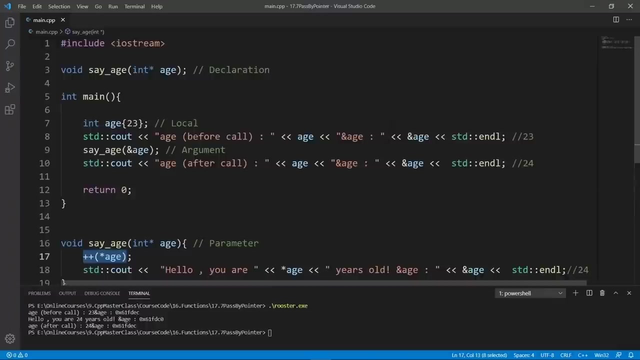 because we just incremented, through our job, The reference operator And after the function call, the age is going to be 24 because we have modified the original variable here through our referencing of the pointer here. This is really all there is about passing by pointer. 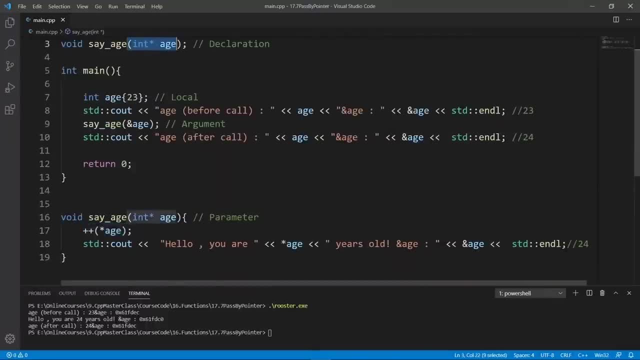 This is the syntax: You have to pass a pointer in the declaration, You have to pass a pointer in the function definition And when you call the function, you have to use the address of the variable and pass that as an argument to the function. 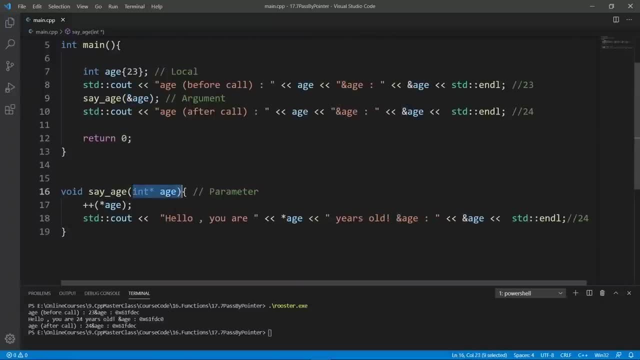 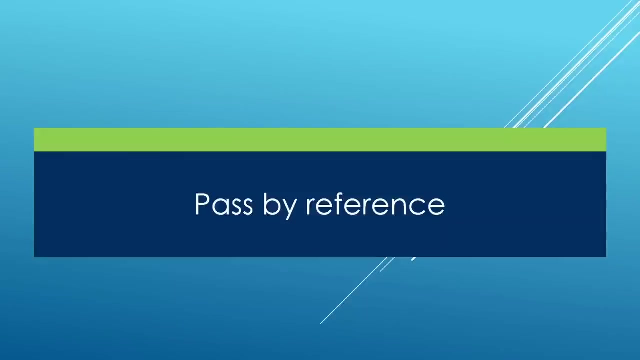 And whenever you need to use the past parameter, you're going to go through the reference operator, like we did here and here in the body of our function. here In this lecture, we're going to see how we can pass parameters to a function by reference. 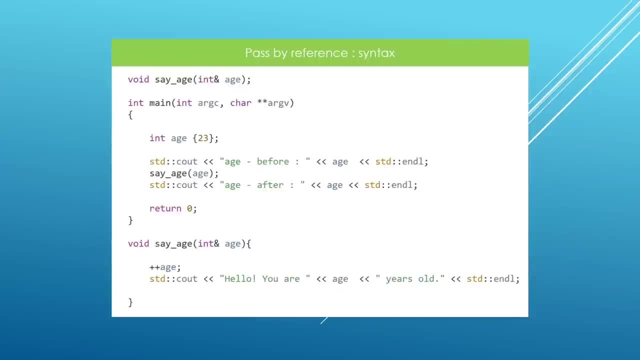 And this is another technique we can use to avoid passing by a value which is going to create a copy. And the syntax is really simple. If you look at the declaration here, you're going to see that we say: if you look at the declaration here, you're going to see that we say: 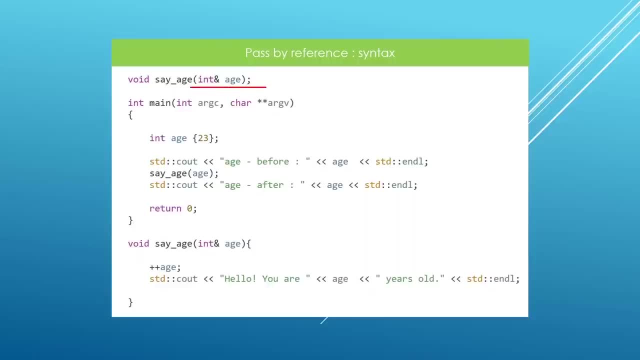 if you look at the declaration here, you're going to see that we say: you're going to see that we say int reference And again, if we hit the definition, we're going to say int reference, as you see here When we call the function. 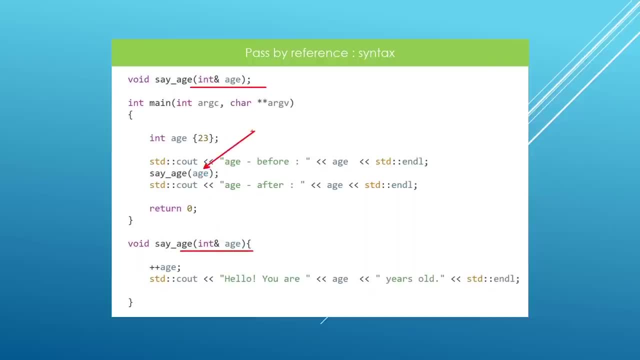 we don't have to pass the address of operator, We just pass the variable, because this is going to be treated as a reference by the compiler And in the body of the function. we don't have to go through ugly the reference and like we did with pointers. 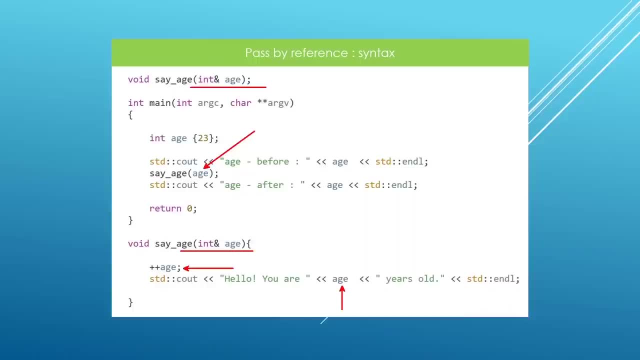 And hopefully you can see that if you want to avoid copies, it's much cleaner. You don't have to use the address of operator when you call the function, like we do here, And you don't have to go through the reference and to access and modify your variables. 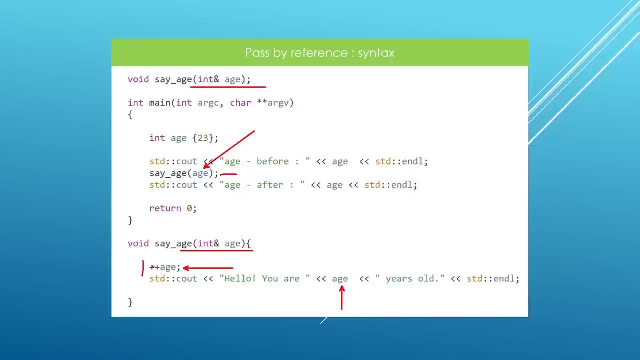 And the modification we do here by incrementing age is going to be seen on the outside because we are going through a reference And the reference is a true alliance to the variable that the reference is referencing. So by incrementing the age here in the body of the function, 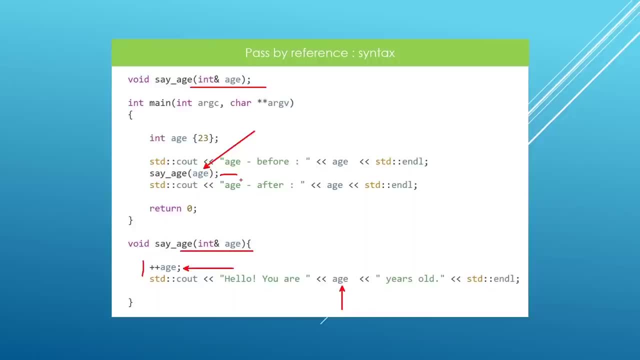 the change is going to be seen after the function call. Before the function. here we're going to get 23.. In the body of the function we're going to get 24, because we just incremented the function, And after the function call we're going to get a 24. 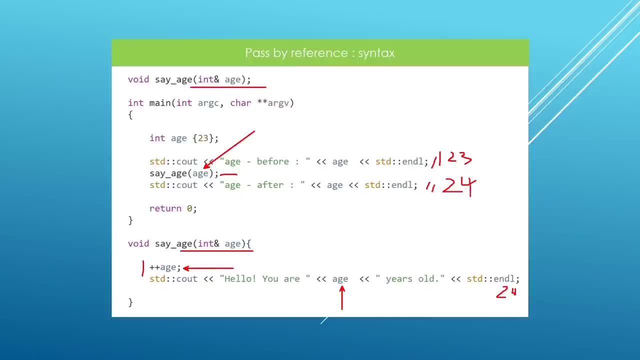 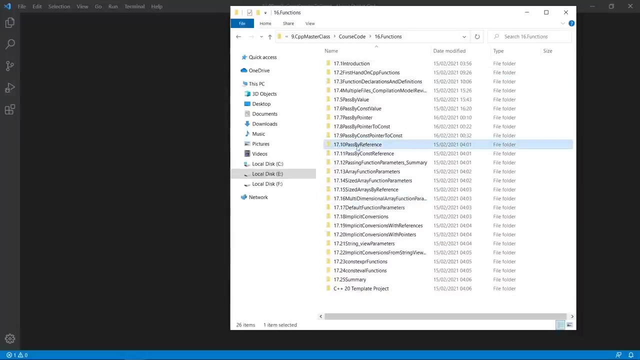 because the change was propagated to the original variable, And the reason is because we are going through a reference here. Let's head to Visual Studio Code and actually play with us a little more. Okay, here we are in Visual Studio Code. The current project is passed by reference 1710 here. 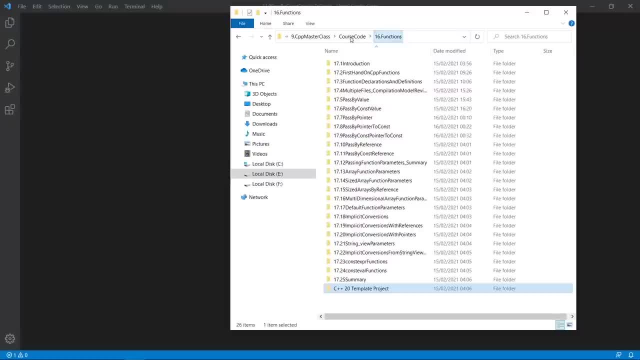 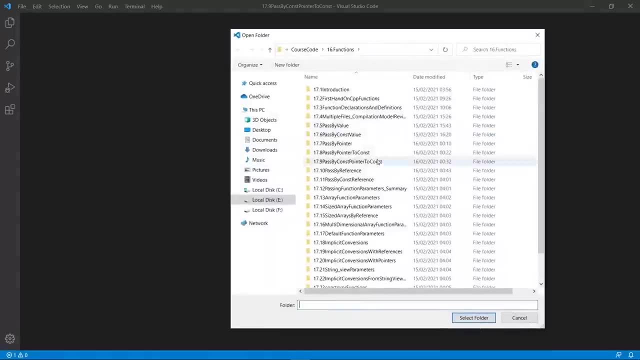 So we're going to grab our template files and put them in place. 1710.. Let's do that And we are going to open this in Visual Studio Code pretty quick. Let's do that. The main CPP file is going to show up here. 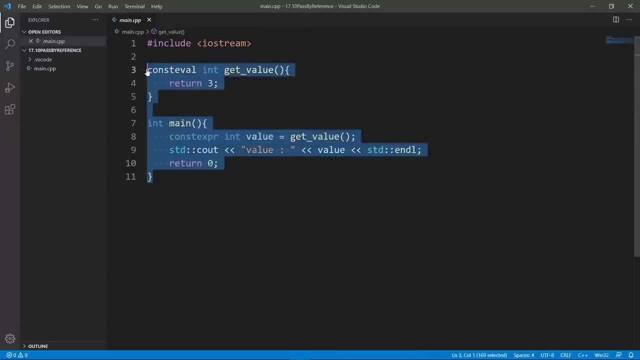 Again, we are going to grab the code from the last lecture and use that as a starting point And we're going to be modifying the signature of our code. And we're going to be modifying the signature of our code. And we're going to be modifying the signature of our code. 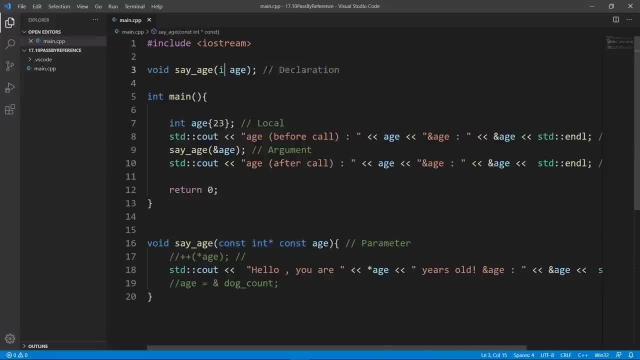 So what we want to do is to pass by reference. We're going to say int reference here. You already know references from a previous chapter And we are going to hit the definition here and do the same thing. So let's say int reference age. 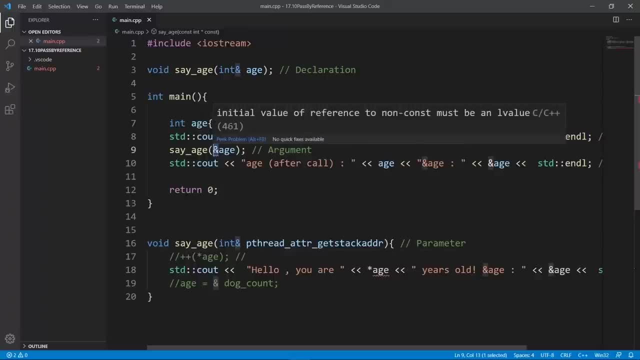 And when we call the function, we don't need to pass the address of operator because this is a reference. We can use it right away. The compiler is going to know that this is going to be a reference to the operator. The compiler is going to know that this is going to be. 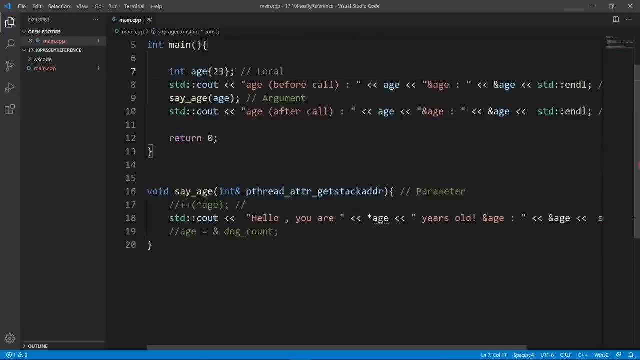 a reference to the operator, And we can use it right away, And we can use it right away, And we can use it right away And in the body of the function. let's take out this last line here. We don't need it. 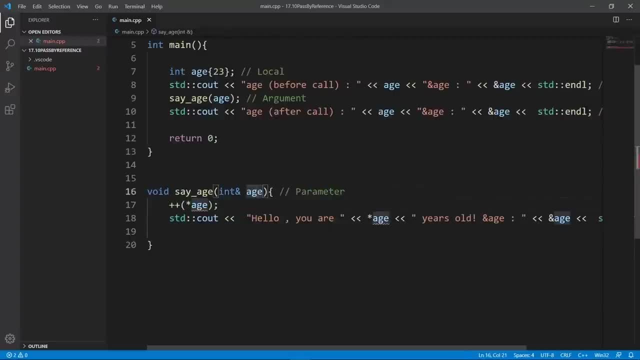 And in the body, when we want to modify the reference, we can do that right away without the referencing. So we can just say plus plus age here, And the changes are going to be propagated to the original variable here because we are going through a reference. 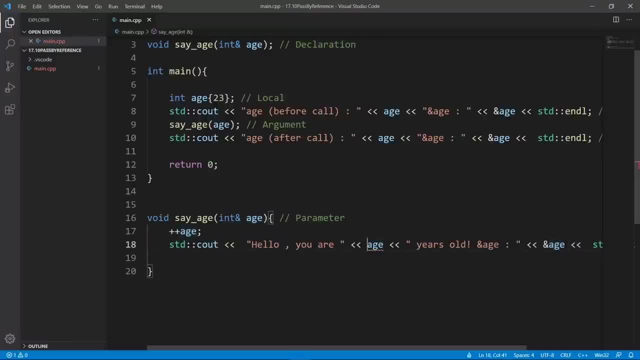 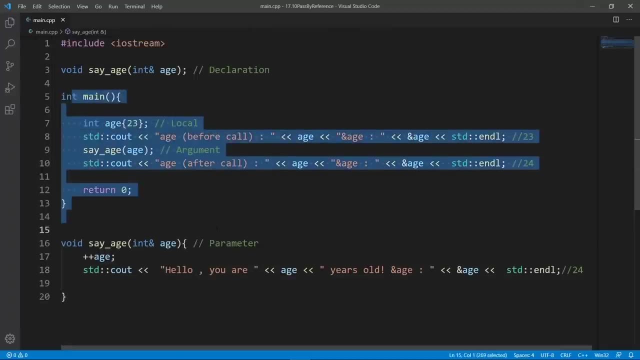 Let's go down and modify this, because this is a reference, We can use it right away. And let's go down And we can close this left pane here, so that we have some more breathing space And you see that Visual Studio Code is no longer giving us any squiggly lines. 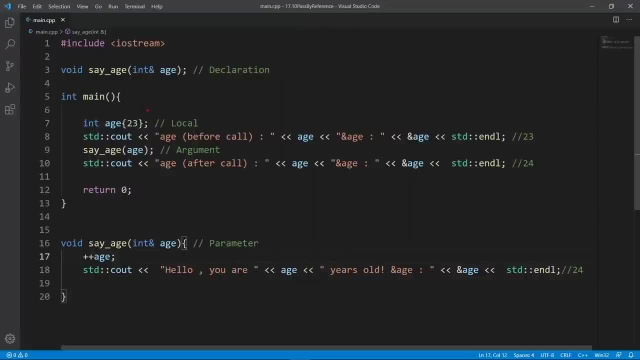 So this must be valid C++ code. Again, notice the syntaxes we are using here. We are passing a reference in our declaration. We are passing a reference in our function definition. here, When we call the function, we don't need to do any address of operator. 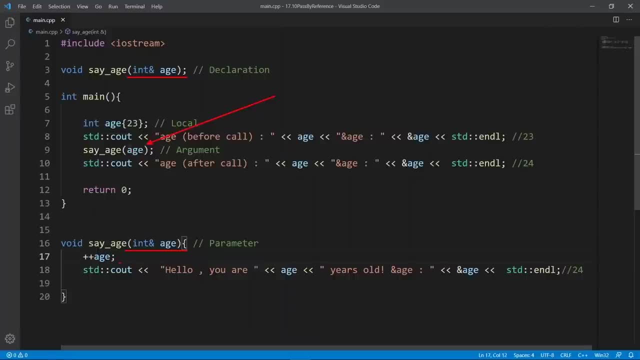 We pass the variable as is And in the body of the function. we don't have to do any de-referencing. We can increment right away or modify the variable however we want. The changes are going to be propagated to the original variable because we are passing a reference. 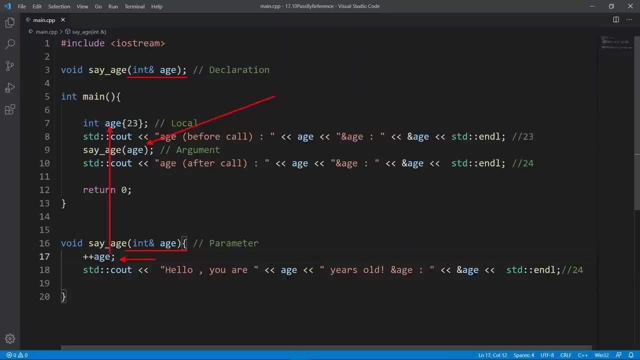 So the incrementation here is also going to affect the original variable that was declared in the main function here. Let's take this out And down here. if we need to use our variable, we're going to just use it right away. We don't need any de-referencing. 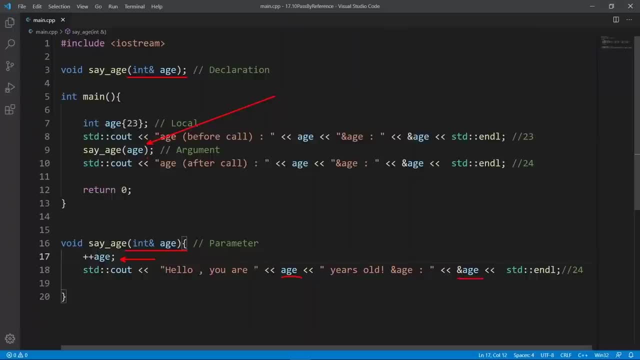 And if we print the address of H here, we're going to see the same address we see on the outside, because this is a true alias. It's going to be referencing the same variable that we have in main here. Okay, now that you have a better idea about this. 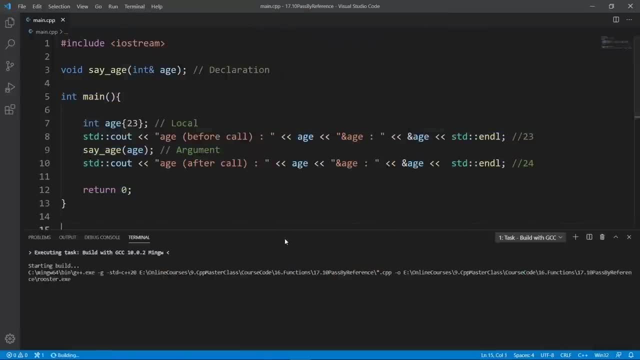 we are going to try and build this. We're going to use GCC, as always. You can see that the build is good. If we bring up a terminal to try and run this program, we can clear, we can run rooster. We're going to see that before we call the function. 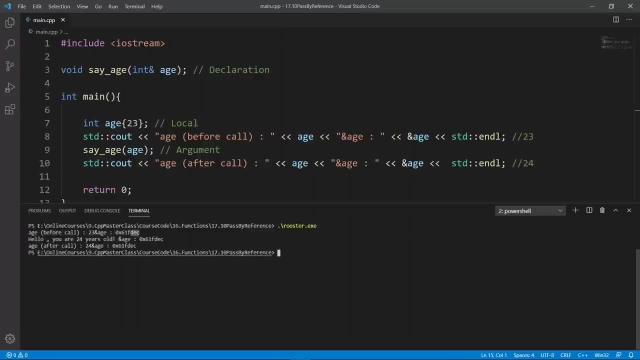 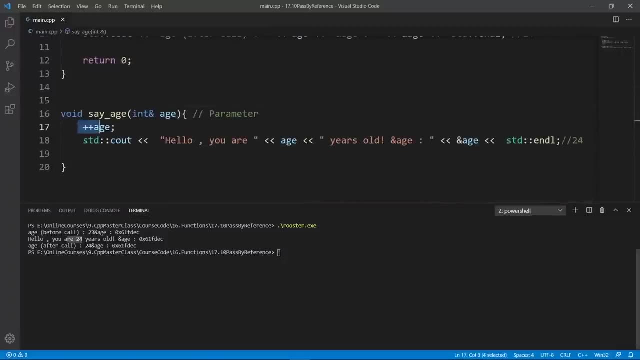 the age is 23,, but the address ends in DEC. When we hit the function, the age is 24, because we just incremented that here. But notice that the address of the variable is the same as on the outside, So we are modifying the same variable. 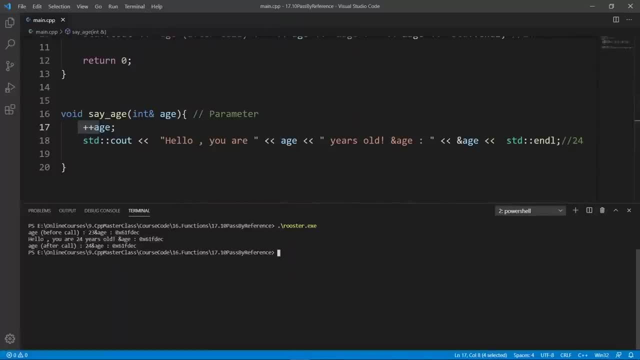 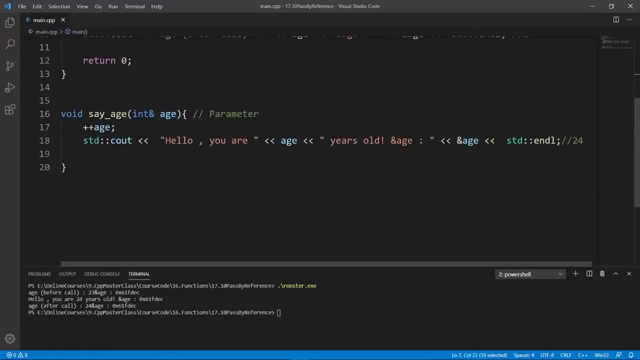 And when the function is done, the age is still going to be 24, because we just modified the original variable through a reference here. Okay, this is the effect of passing by reference. You can use a clean syntax to modify the original variable. 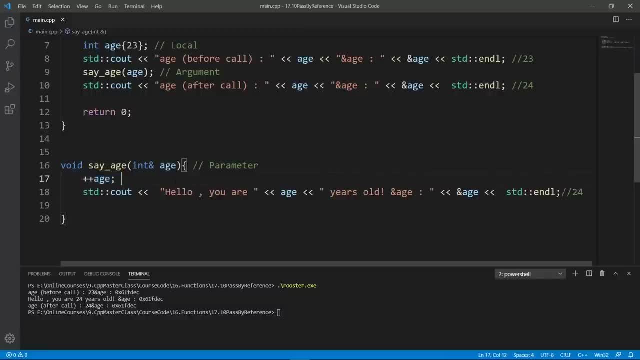 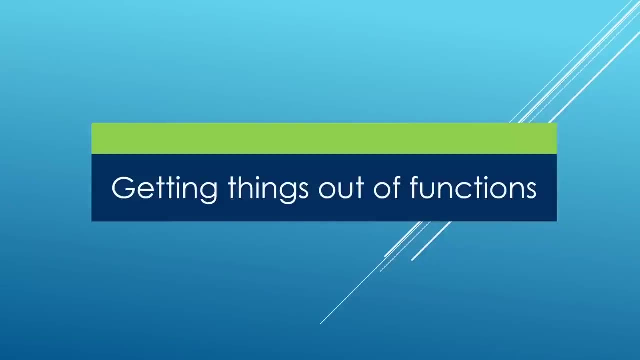 in your functions, And this is going to avoid copies, like we have seen when we were passing parameters by value a few lectures back. I would like to welcome you in this new chapter, where we will be focusing on how to get data out of functions. 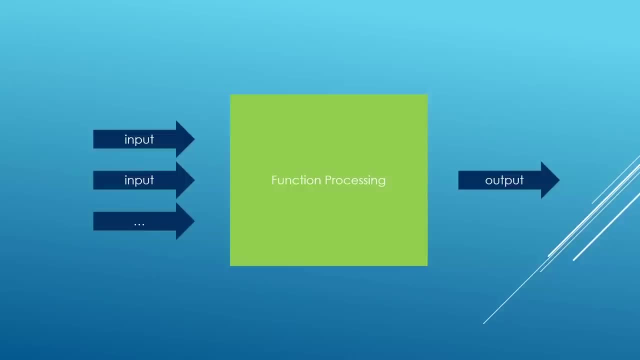 Again, the model of the function is really what you see here. It is like a machine and you can give input to that machine and you expect to get something out of that machine. This chapter is going to focus on this part here. 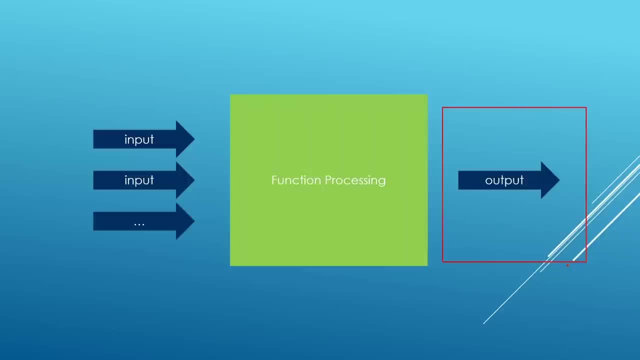 and we're going to see the different facilities offered by the C++ programming language to get output from functions And we are going to start in the next lecture and see how we can use input and output parameters. Go ahead and finish up here and meet me there. 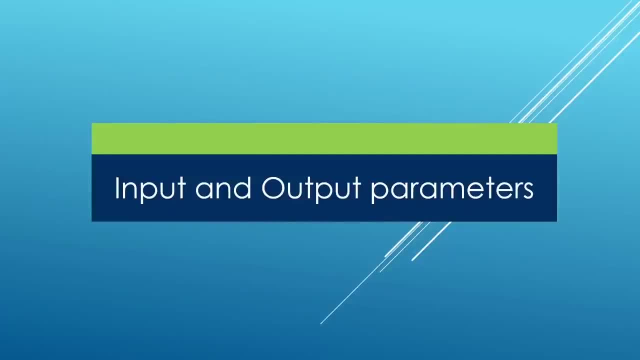 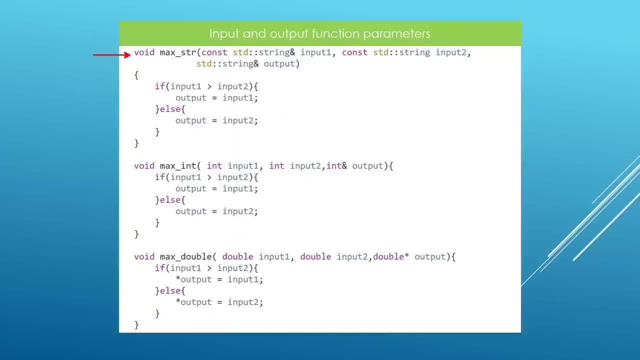 In this lecture we're going to see how we can use function parameters to get data out of the function. Here is a simple example and we have three functions here. We have maxstr, maxant and maxdouble And you notice that we have three parameters. 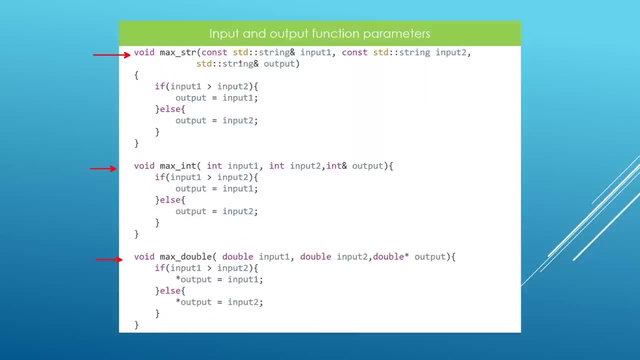 for each of these functions. The first two parameters are going to be input- They are going to get data in the function- And the third one is going to be the output parameter, and it is going to get data out of the function. Let's focus on maxstr. 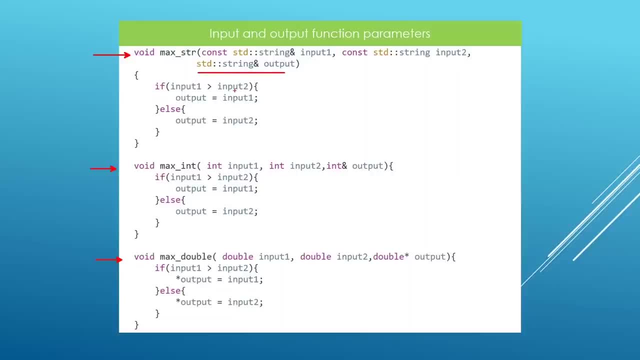 And we're going to see how we can use this parameter to get data out of the function. We have maxstr here and we're going to use maxstr here And we're going to see how we can use maxstr here and really drive the point home. 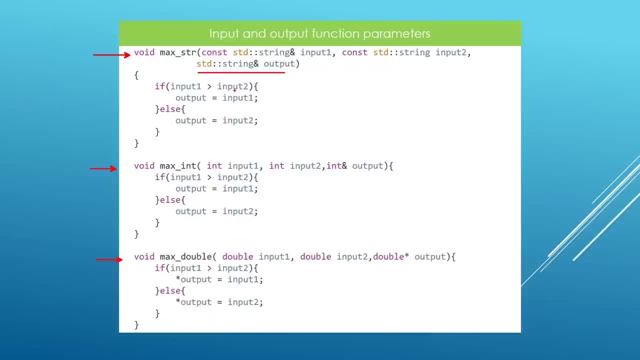 The key idea here is that for the third parameter, we are using a modifiable reference, And if we use a reference, the changes we do inside the function are also going to be visible on the outside, And we explicitly left out the const that we have. 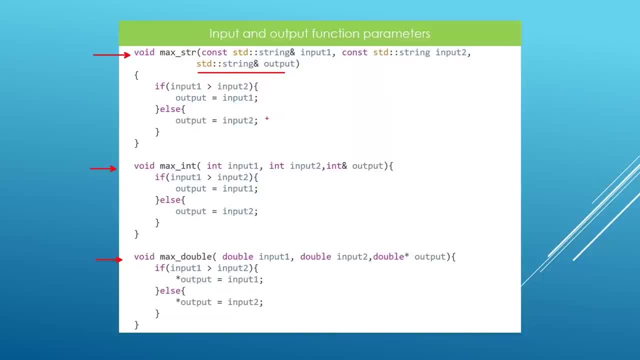 here If we marked the third parameter as const. we would get a compiler error if we tried to do something like this and assign something to the output parameter here. So the main purpose of this function is to compute the maximum between these two strings. 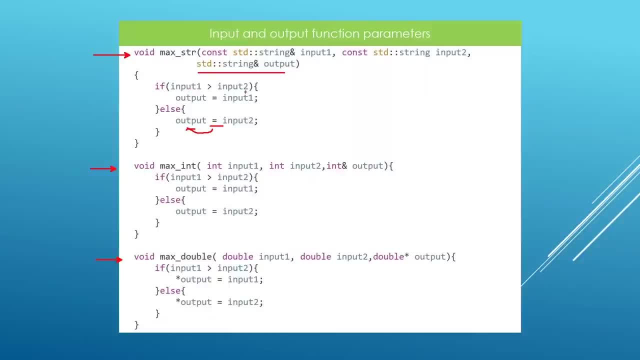 We are going to say if input one is greater than input two, then input one is going to be our maximum And we are going to store that in our output parameter here. If input one is not greater than input two, then input two is our maximum. 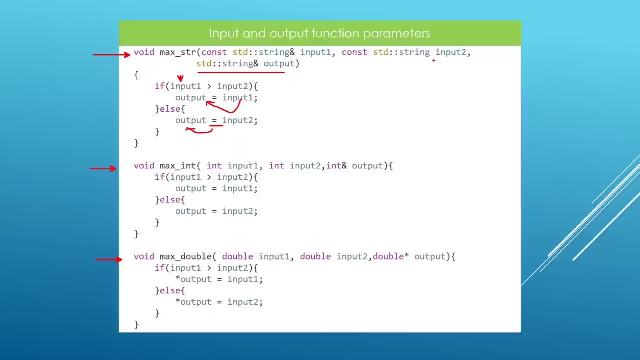 We're going to store that in our output, And whoever has access to input two outside the function is going to see the changes that we are making in the body of the function. This is really the technique we can use to send output from the function and make it visible when the 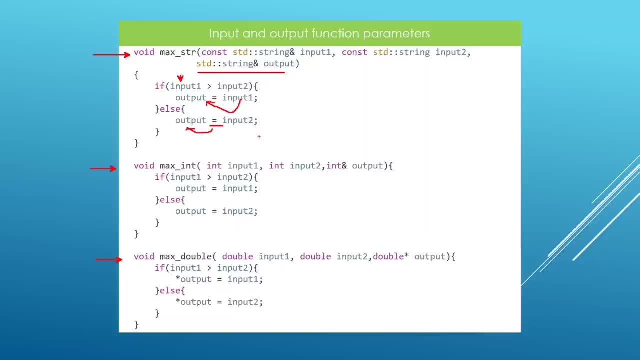 function has returned. And again, the key idea is that we set up the function in a way that the changes we do inside the function are going to be visible on the outside. Good luck. and we are able to do that because output here is a reference. this is: 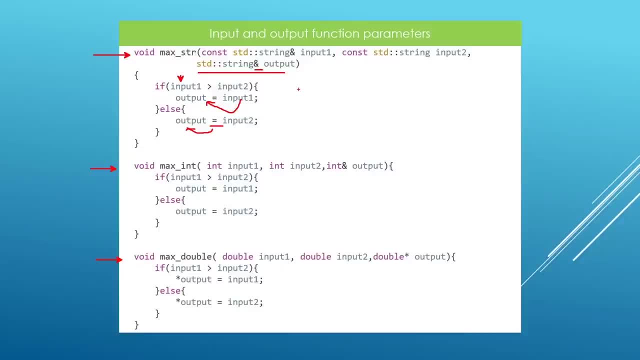 really key. we have used references here, but we can set up the same thing using pointers, because we have seen that with pointers we can also make our changes inside the function visible to the outside. the two other examples here are really extensions of the same thing. we have two input variables: input one and. 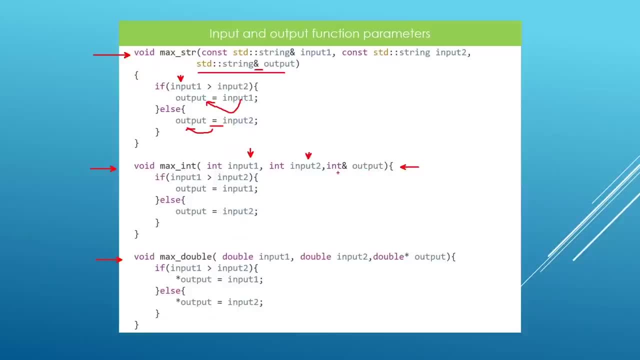 input two and output is going to store the output from the function. you notice that output is a reference and because of this the changes we do in here are going to be visible when this function has returned. and we do exactly the same thing on max double here, but you see that it is using a pointer. okay, I really 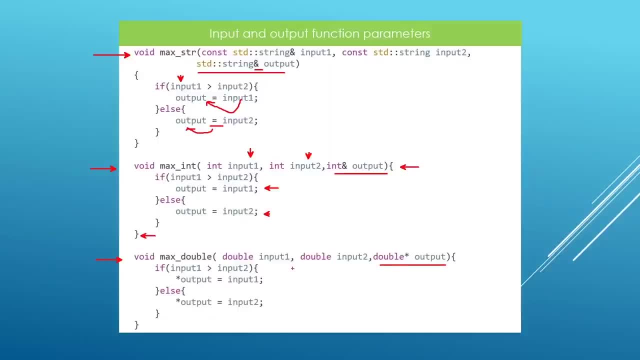 wanted you to see this. so inside we're going to try and figure out who is the maximum, and if input one is the maximum, we're going to write that here, and if input one is the maximum, we're going to write that here, and if input two is the maximum, we're going to write that in our output variable here. 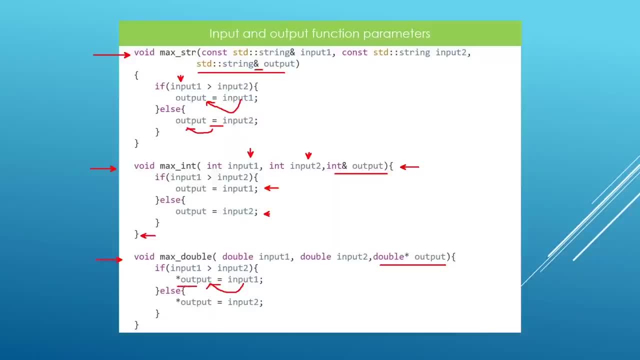 and you notice that we are the reference in here, because this guy is a pointer and if input two is our maximum, we're going to write that in our output variable here. one thing I don't think I explained here is that we have a const std string reference here for max std r and the reason is that the input 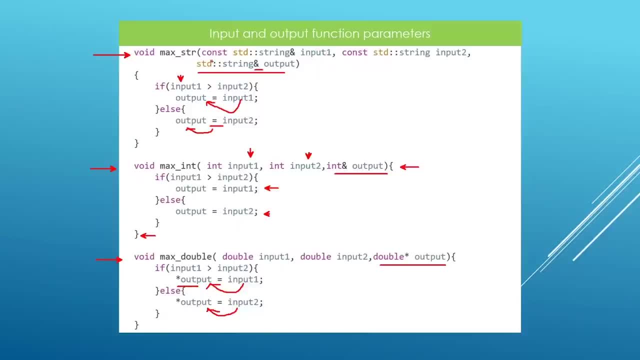 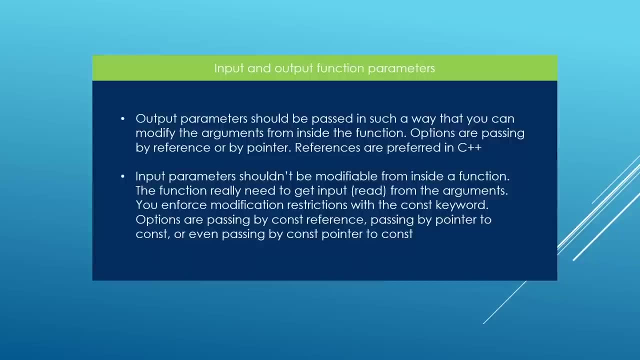 variables aren't really meant to be changed. that's why we mark them as const, and if you want to modify them, you can do that by using the const- std string variables. that's why we mark them as const- std string. okay, this is really the big idea we are playing with in this lecture, using 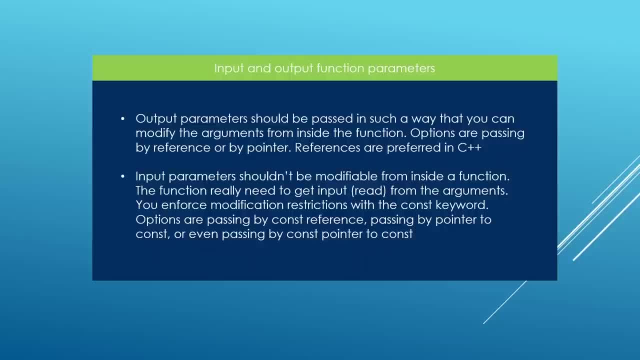 function parameters as a way to output data from the function, and here are a few ideas you should keep in mind. output parameters should be passed in such a way that you can modify the arguments from the inside the functions, and we have seen that we have two ways to do that. we could either use references or 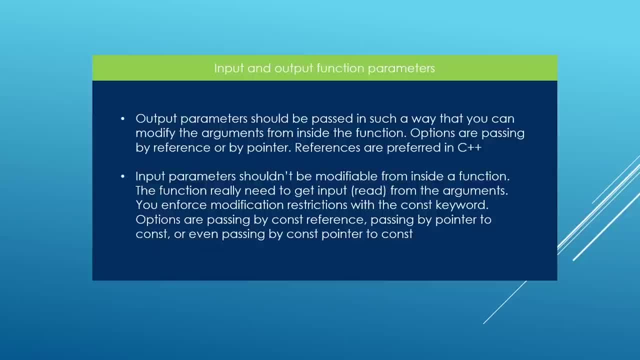 even use pointers, but references are you should prefer. in modern c++, input parameters shouldn't be modified. they are meant to just get data in the function and that's why, in most cases, you're going to see that they are marked cost. okay, now that we have seen all these ideas, i think it is time we headed over to. 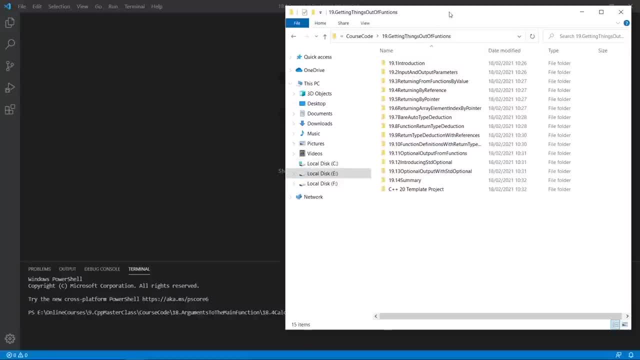 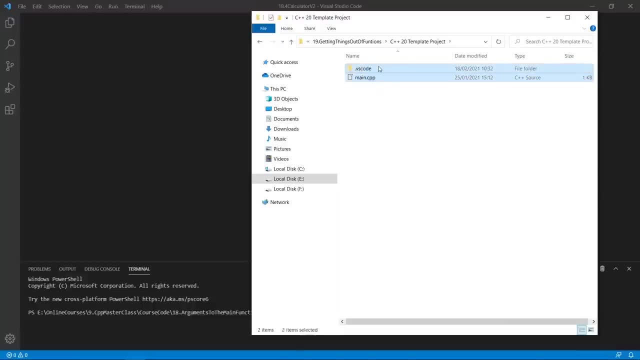 visual studio code and actually played with them. okay, here we are in our working folder. the current project is input and output parameters. we are going to grab our template files, like we always do, we're going to put them in place and we are going to open this guy in visual studio. 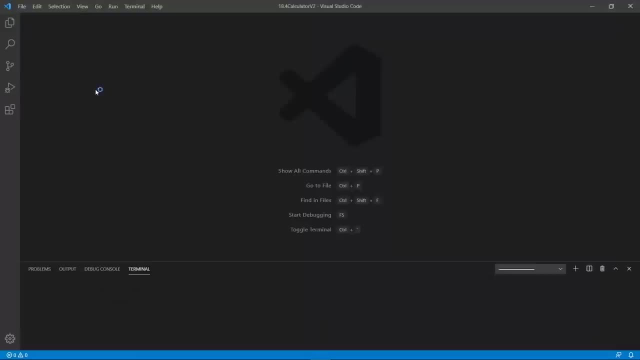 code. we're going to just drag it and drop on top of visual studio code here and it is going to open up. we have our main function here. we can close the pane here and clean the file up a little bit. we're going to remove what we don't need here and we're going to have a bare main function. we can. 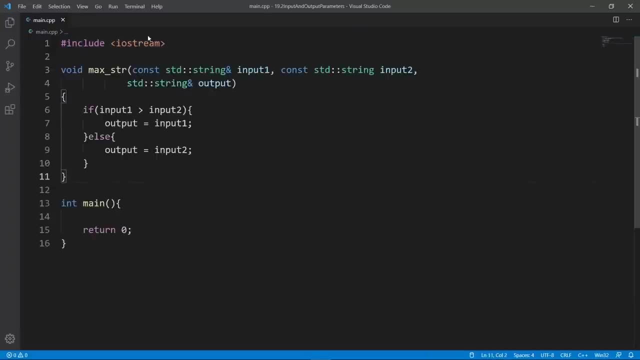 play with here. the first thing we're going to do is to put in our max str function. it is nothing special. we just have two input parameters and one output parameter. the output parameter is going to be what we use to get output outside the function, and inside we're just going to compute the maximum if input 1. 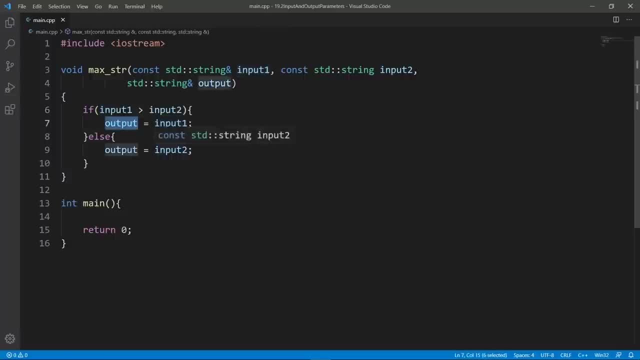 is the maximum, we're going to write that in our output parameter. if input 2 happens to be our maximum, we're going to write that in our output parameter because our output parameter is a reference. the changes we make inside the function are going to be visible on the outside because 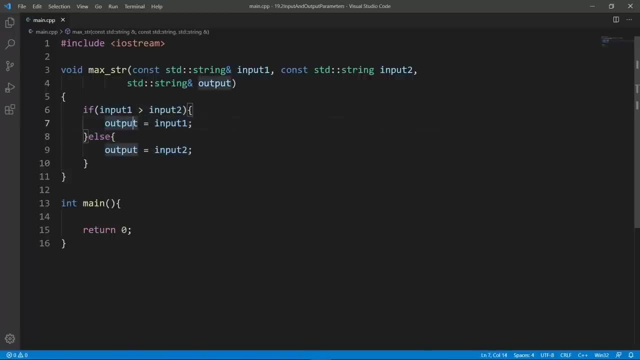 we will be working on the original variable through the reference, which is really a true alias here. okay, now that we have the function set up like this, we can head in the main function and try it out. we're going to set up three variables of type std strand. i think we should include. 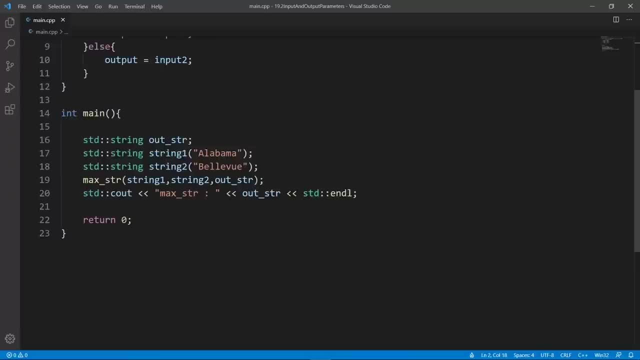 the string library here. let's do that and we're going to have an out string which is going to be our output variable, and we have two input strings: one is initialized with alabama, the other is initialized with bellevue, and we're going to call our max str function here you. 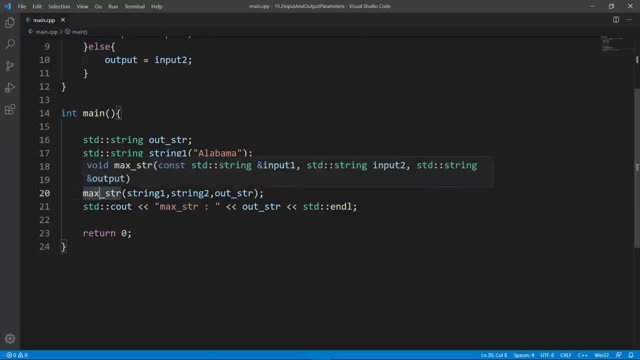 notice that it's not going to be using the return mechanism. we're going to be grabbing the output from this function using an output parameter, which is going to be our out str variable here. okay, once the function is done, we're going to have the maximum stored in our out str variable. 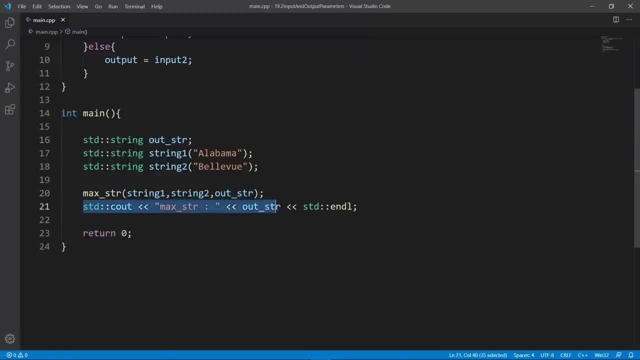 here and we can print it out. now that we have this set up, we can actually try and build this. we're going to use gcc. let's do that. the world is good. we can bring up a terminal and clear and run rooster. now you see that the maximum is going to be bellevue. let's. 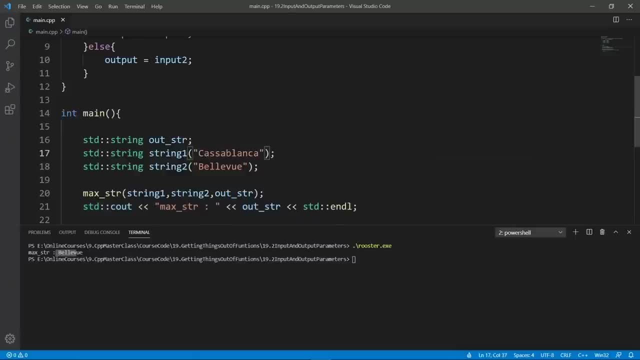 try and change this to casablanca- why not? and we're going to see that the maximum now is going to be casablanca and our function is going to be smart enough to store the maximum in this output variable. here let's build again. the world is going to be good. i'm going to clear and run rooster. 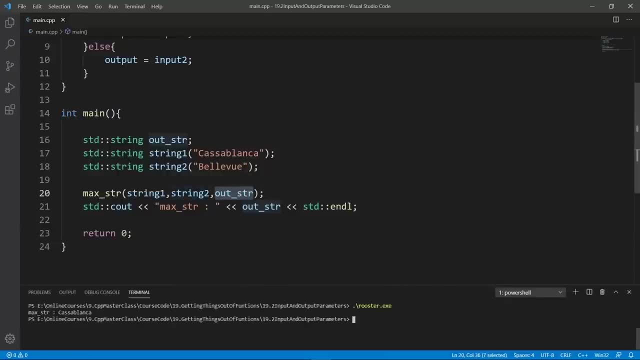 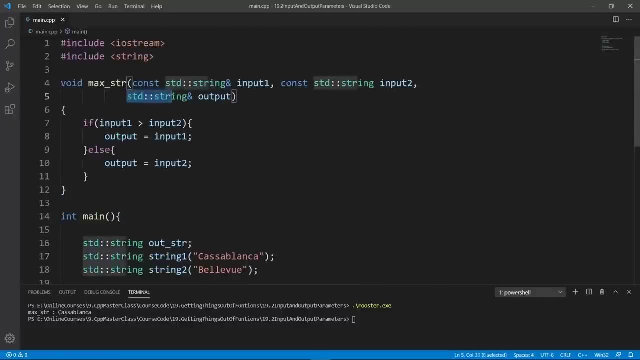 the maximum is casablanca. hopefully you understand that we are able to make the changes in the function persist because our output parameter here is passed by reference. this is a true reference and any change we do to the output parameter here is going to be visible in whatever variable you passed. 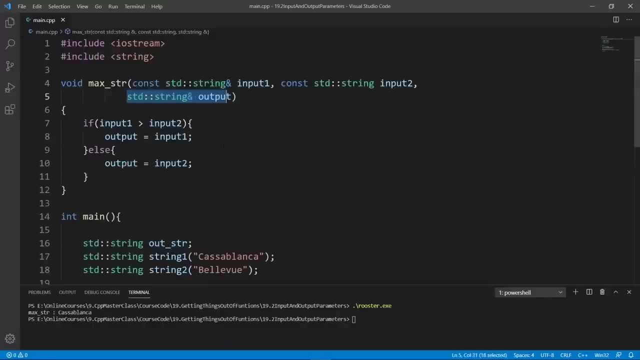 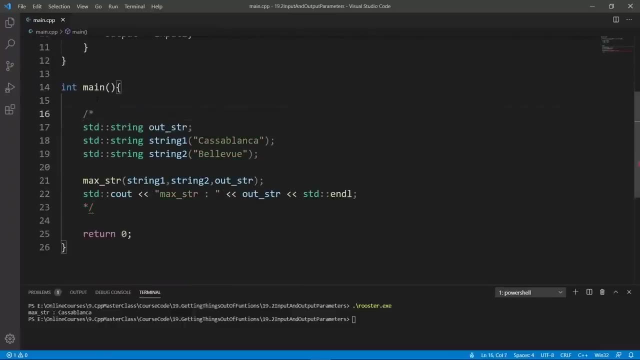 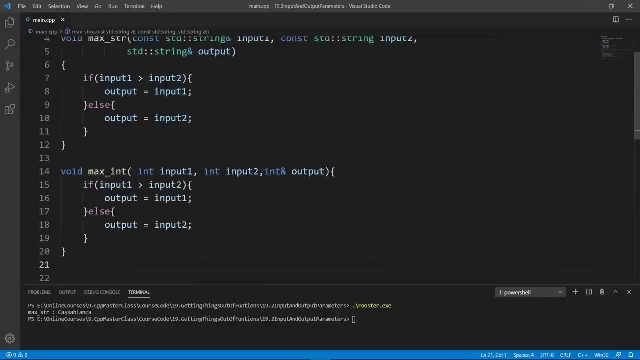 as an argument for this third argument here. this is what is making this work. now that this is working, we're going to comment this out and put in another example for you to play with. the next function we're going to play with is going to be max and, as you see here- and it is very similar to our max sdr, but you notice that. 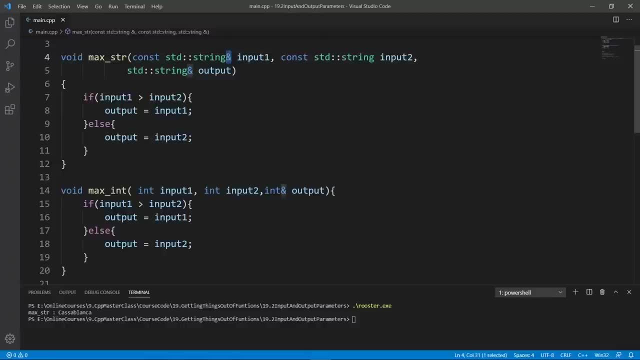 our inputs are no longer references because we don't really mind copying fundamental types in c plus plus. they are small in memory so copying them is really cheap. we can pass them by value and this is not going to be so wasteful in our program. but the first parameter must be passed by reference because we want to use it as. 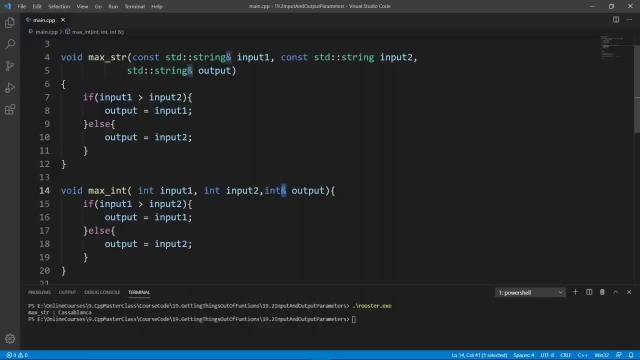 an output parameter and we're going to use it to get output from the function, and the way we're going to do that. we're going to write whatever variable is the maximum in our output parameter and the changes are going to be visible on the outside. now we are going to head over in our main. 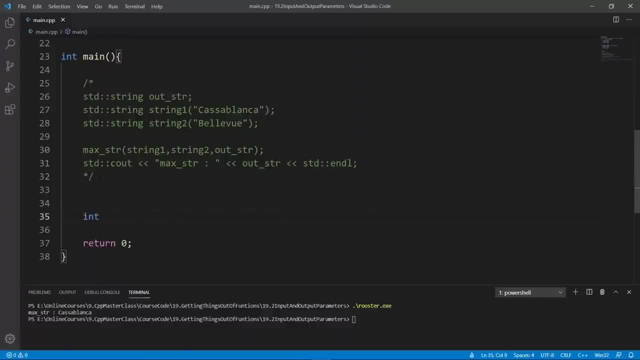 function set up a few variables and play with us. so we're going to say and out, and this is going to be our output variable. and we're going to say input one, let's say in one, and we're going to initialize this with a 45, why not? and we're going to say and in two, and we're going to initialize: 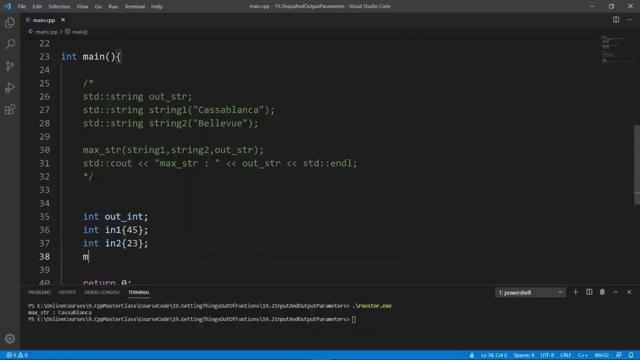 this with 23, why not? now that we have this, we're going to say max and and we're going to put in our input. we're going to say in one and in two. then we're going to say out and as our output variable. now that we have this, we can actually print out whatever number is the maximum through. 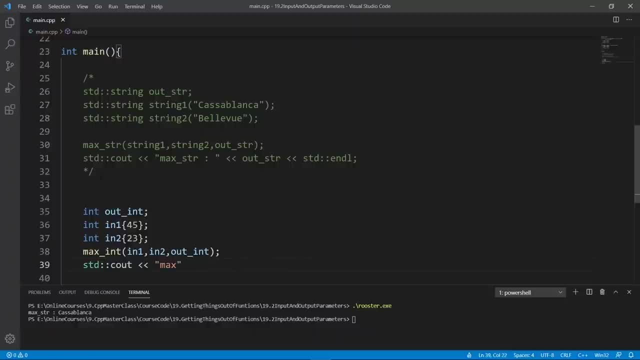 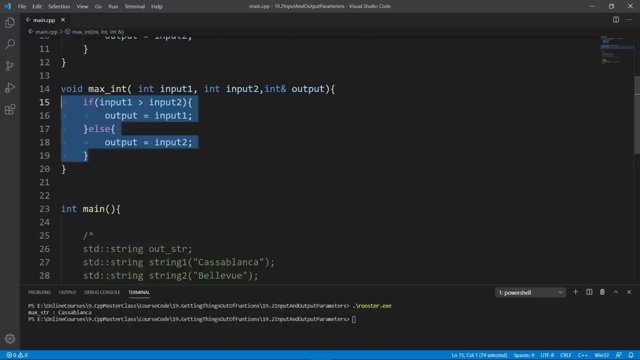 a statement like this, really simple: we're going to say max and and we're going to say out and that's where it is going to be stored. and we are able to do this because, again, the third parameter here is passed by reference and any change we do and the function here is going to stick, even when. 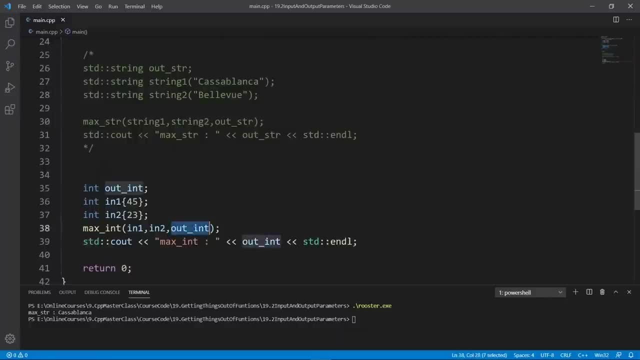 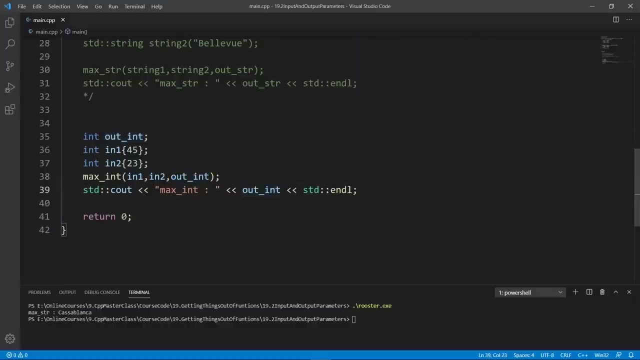 the function here has returned and we're going to have that stored in our third parameter here, and this is a really common technique, especially in code that has to interface with c code out there from c plus plus, and you really need to be aware of this now. 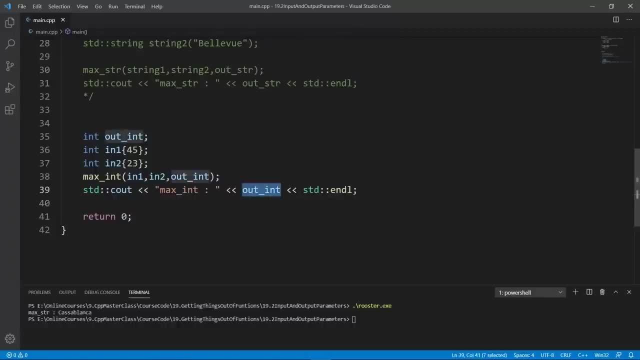 if we run this program, we're going to see our maximum printed out and it is going to be stored in our out variable here. let's do that. we're going to use gcc to world- the world is good, you can clear and run rooster- and you're going to see that the maximum is 45 if we change and store. 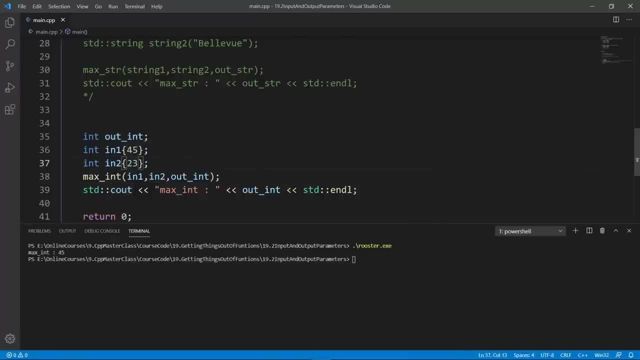 our maximum in into here. and for example, let's make this a 700 and 23, let's weld again to take the changes into account in our roosterxe binary. we're going to clear and run rooster and you're going to see that that's the maximum here we are able to grab. 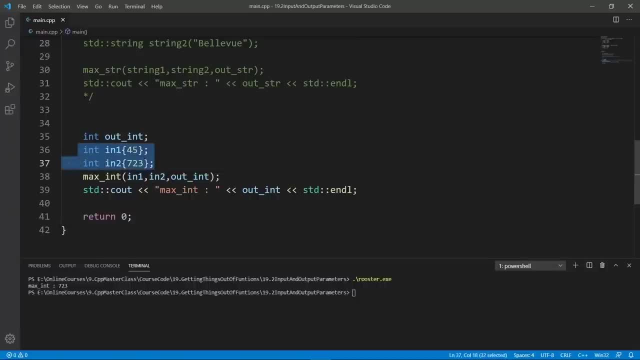 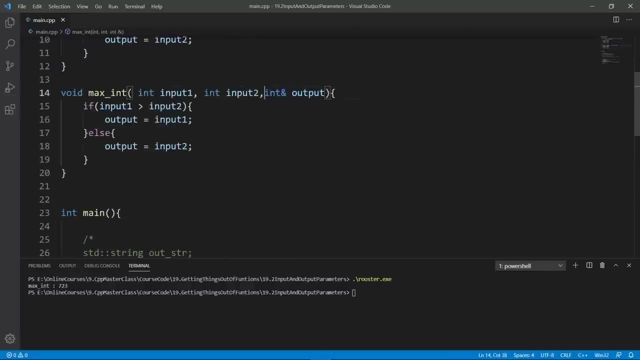 whatever is the maximum from these two input parameters and store that in our output parameter here, because we are passing that third guy as a reference. this is really important. we have seen that we can use references to make changes we do in the function stick and be visible in outside variables. but we can also use pointers. 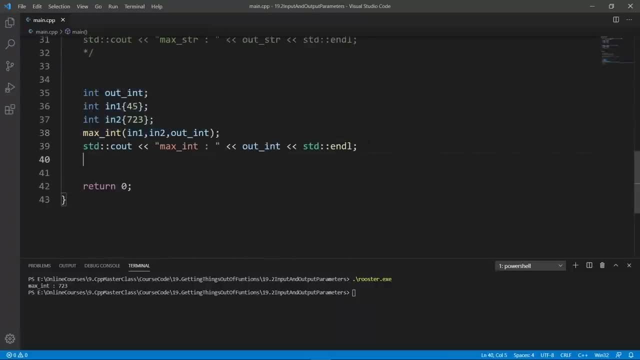 and i am going to show you an example of how we can do that. first, we're going to comment this out because we don't want noise output in our program and we are going to go on top and set up a max double function which is going to grab our output using pointers. the name of the function. 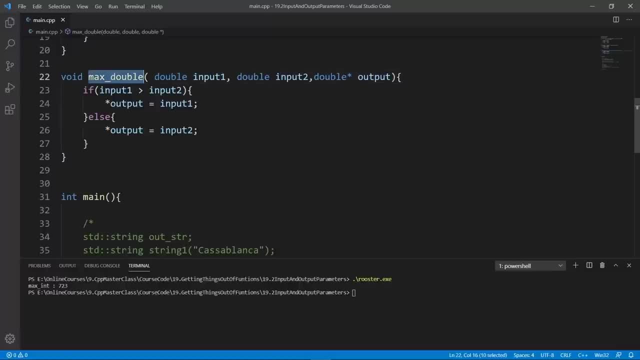 is max double. it's not going to return anything and it is going to take two input parameters, input one and input two, and it is going to tell us whichever of these two is the maximum. the maximum is going to be stored in our output parameter, but we are using pointers to make the 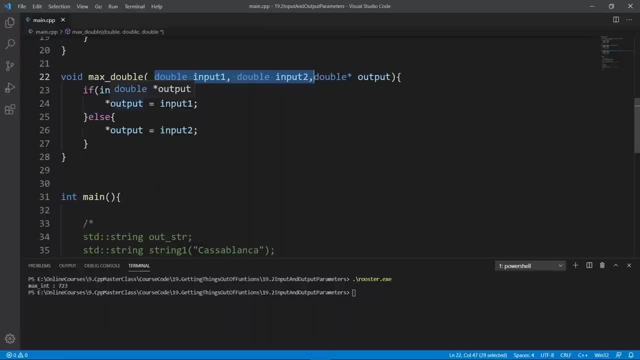 changes inside the body of the function stick and be visible on the outside of the function. so we are going to the reference here, because the third guy here is a pointer, and we're going to store in whichever is the maximum and when the function returns the maximum is going to be visible on the outside. 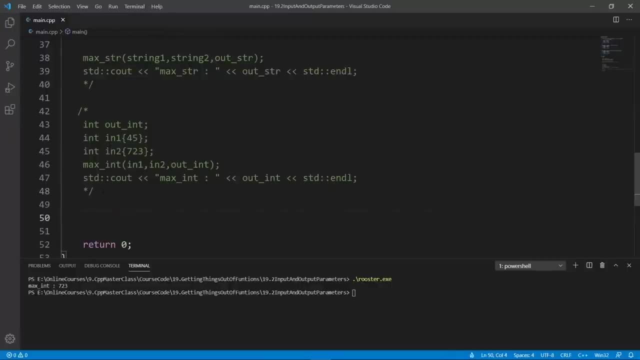 the maximum is going to be visible on the outside, so let's go down and try this out. we're going to say double out, double, and we're going to set up our input here. we're going to say in double one and we're going to make this 45.8. 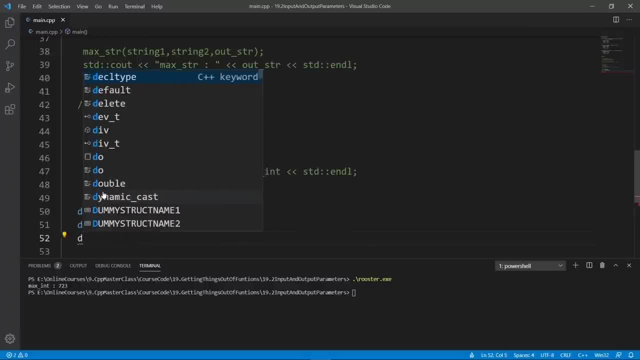 why not? and we're going to do a second input parameter and int. we should say n, not end- sorry for this- in double, for input double. so we're going to say double two and we're going to initialize this with 6.9, for example. we can really put in anything. 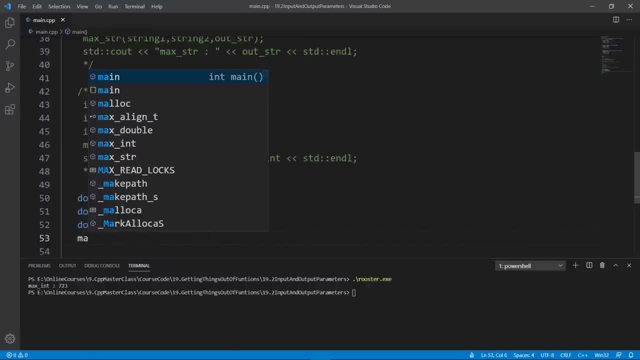 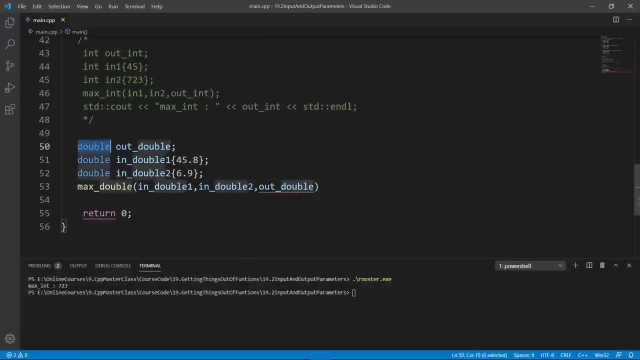 now that we have this, we can call our max double function. let's do that. we're going to say max double. we're going to say in double one and in double two. let's do that and we're going to have out double as our output parameter. and, uh, because it's a pointer, we need to pass this guy as an. 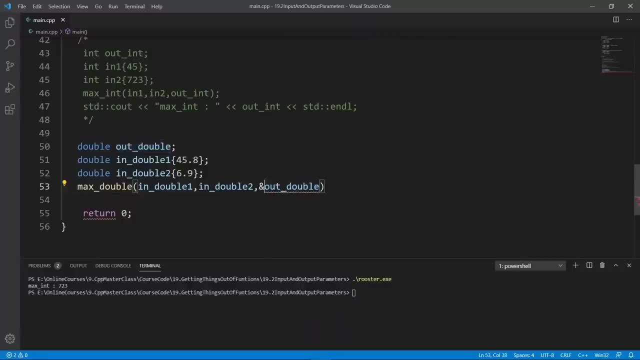 address. so we're going to say address of out to double here. that's how we're going to be able to manipulate that inside the function here. once we do this, we are going to have our maximum stored in out double and we can print that out. so we're going to say stdc out max double and we're 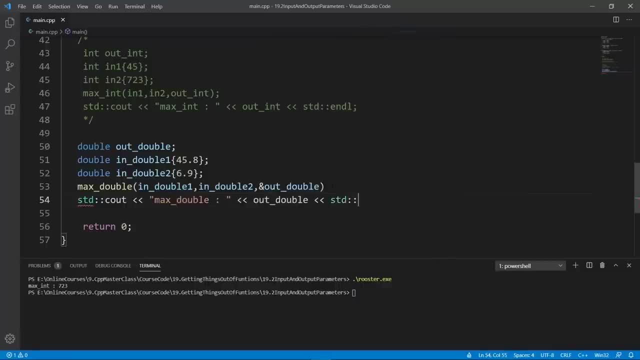 going to say: and we're going to say out double std, endl. and if we bolt, why do we have a squiggly line here? we don't have a semicolon at the end of our function called here, so we're going to build with gcc as always. you're going to see that the world is good, we can clear and run. rooster max is 45.8. 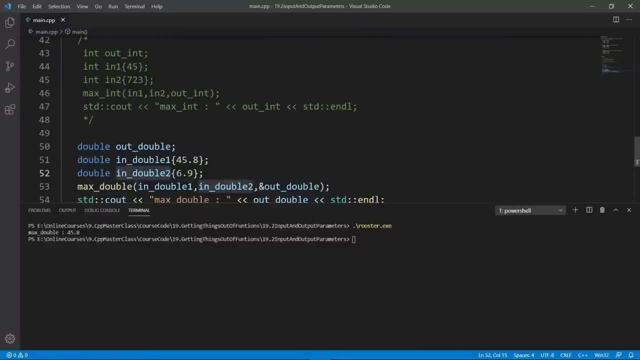 if we change and store it our maximum- and in double two here we can change this guy to 76.9- we're going to world and see that we are actually grabbing the maximum, regardless of the variable in which it is stored. if we run roaster, we're going to have our maximum and this is working exactly as we want this is. 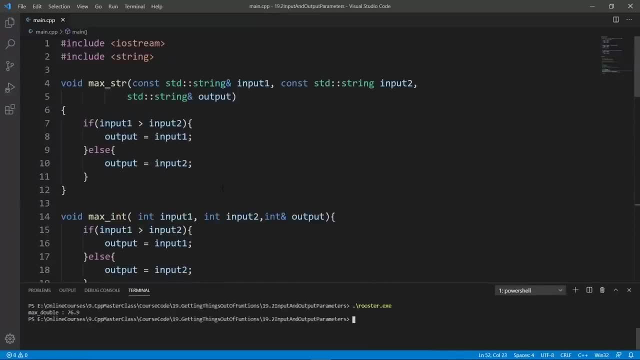 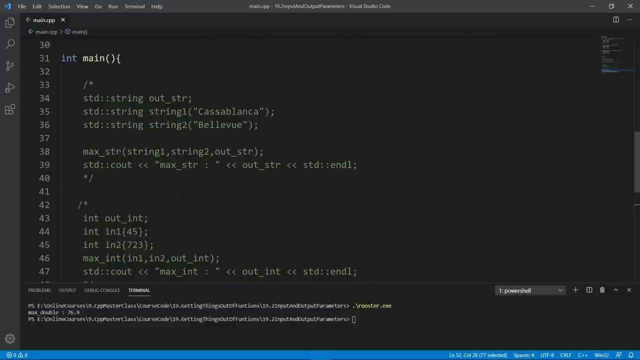 really all we set out to do in this lecture: showing you how you can use references to use parameters as output channels for data to get outside of the function and be used in variables that are outside the function. here i really hope this makes sense and this is a 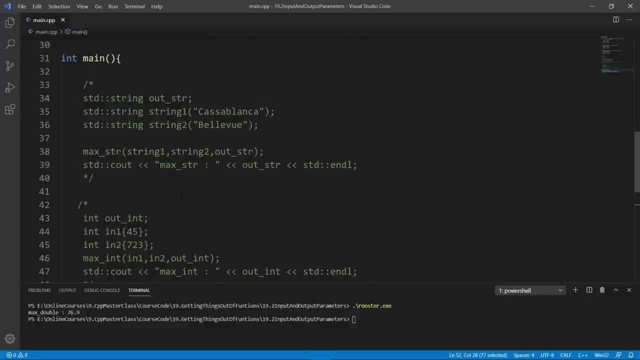 technique you need to be aware of. we're going to see other techniques to do the same thing and, starting in the next lecture, we're going to see how we can return from functions. for now, i hope you found this lecture interesting. we are going to stop here in this one. in the next one, 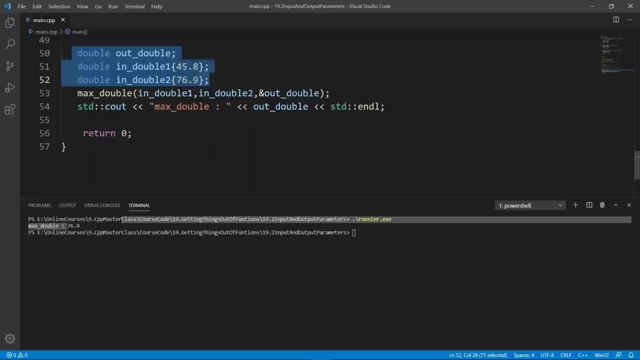 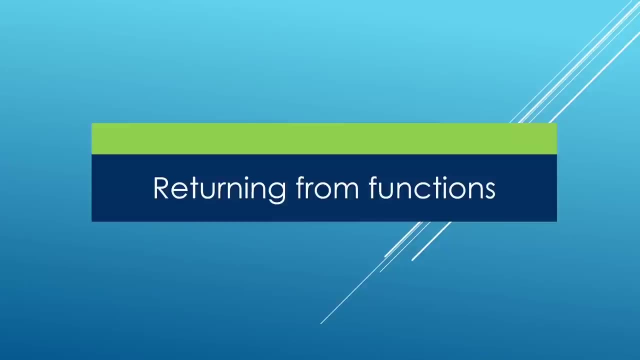 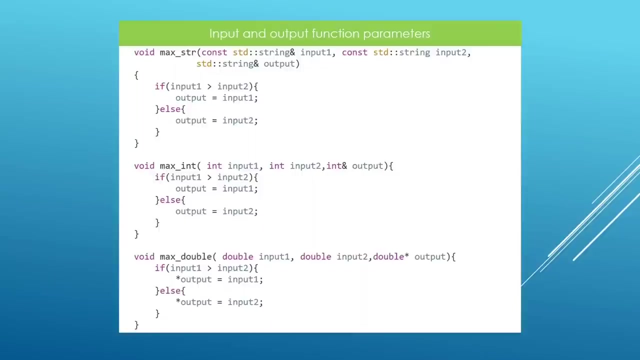 we're going to see how we can use the return mechanism to get data outside our function- go ahead and finish up here- and we can see how we can get data outside of the function through the return mechanism, and this is going to be an alternative to the way we have been doing things in the last lecture, where we used function. 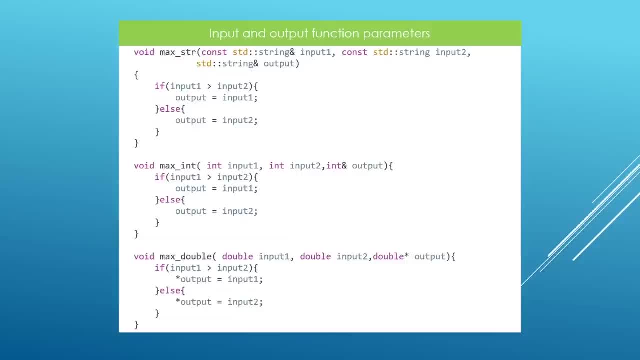 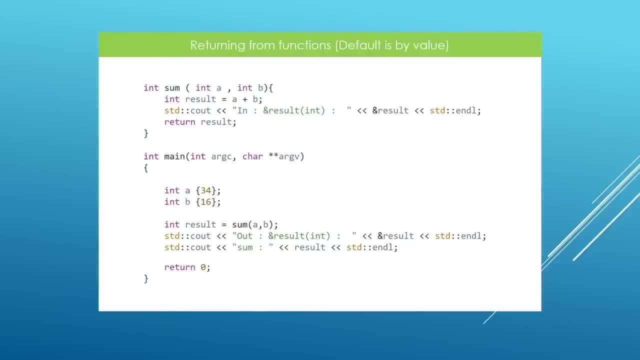 parameters as channels to get data outside of the function. let's look at a simple example of how this is done. here we have a simple function called sum. the function is going to return and and it is going to sum up the function, and the function is going to return the function. 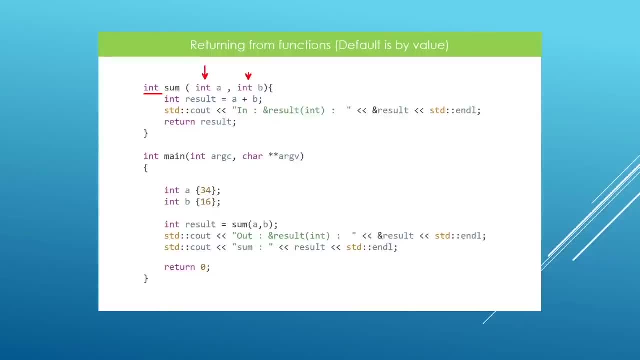 and now we need to do the same thing. we're going to do the same thing here. we're going to sum up two parameters that we pass to it, and a, and and b if we get inside the function. we're going to do something really simple. we're going to set up a new variable which is local to the function. 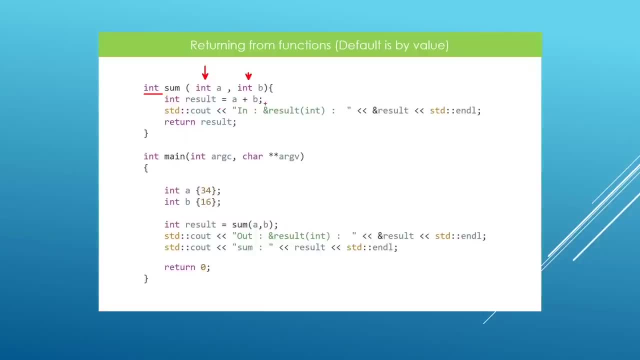 we're going to call that reserved. it's going to be the same type as our input parameters and we're going to add up a and b and store the results back in our reserved variable here. once we have this, we're going to return this for this variable to be visible by whoever called this. 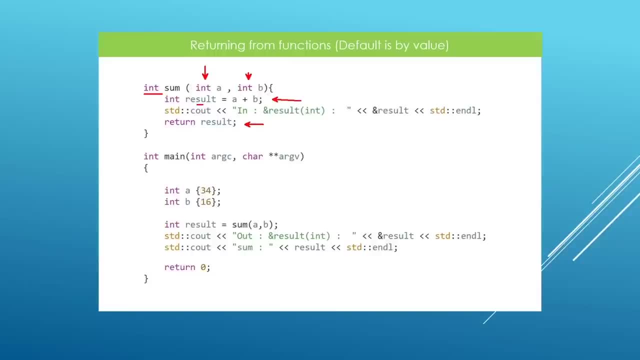 function. and now what we should note is that this variable is local to this function here and it will be destroyed the moment we hit the end of the function here and the function terminates. so if we go in main here, we're going to try and see an example of how we can call this function. 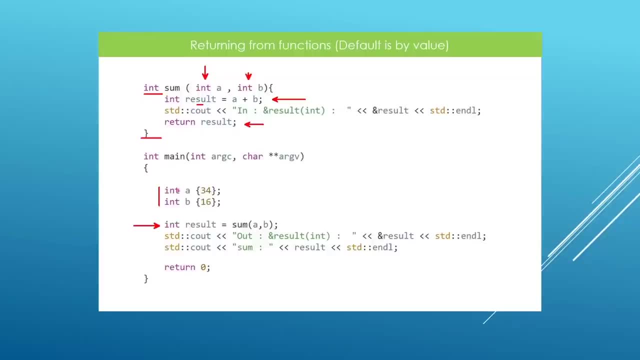 we have two variables, a and b, and we have a new result variable set up in the main function. please note that this variable is very different from the variable we have function here because they live in different scopes. okay, we are calling our sum function here and we are passing it to arguments in the form of a and B here. 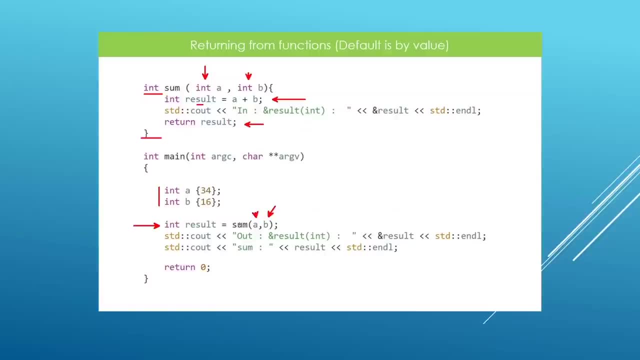 the function is going to compute our sum and it's going to return it and we're going to store that back in our local variable to the main function here. the reserved variable here again is local to this main function. okay, once we call this function, we're going to have our results stored in here and if we print, 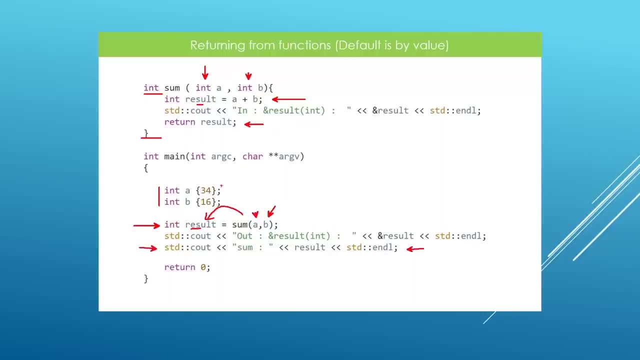 like we do here. we're going to see it printed out on the console. in this case it's going to print 50, because 34 adding 16, that's going to be 50. but one thing I want you to know is that this is going to return by value and what we mean by. 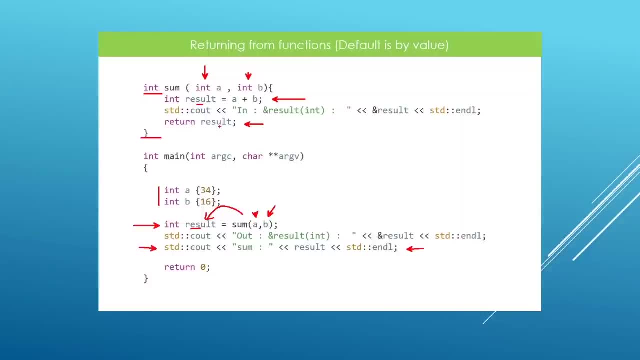 this is that we're going to copy whatever we return here and store a copy of that in this reserved variable that we have in the main function and we're going to prove this notice the STDC out statement we have here. and we're going to prove this notice: the STDC out statement we have here. 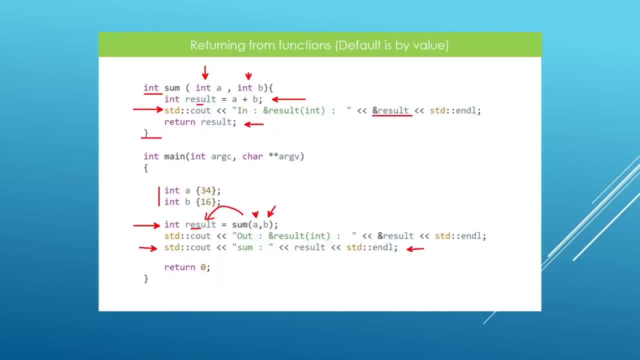 this is going to print the address of this local variable and once the function terminates, we're going to try and print the address of this reserved variable in the local scope of the main function and we're going to see two different addresses and hopefully this is going to prove that we are returning. 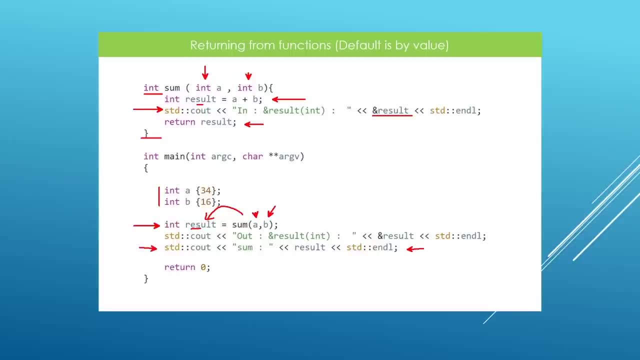 a copy. it's not the original variable that we have in the sum function here that we are returning. okay, hopefully this drives the point home that we can use the return mechanism to get data outside the function and we're going to grab the result in our result variable here and we're going to use it however we wanted. 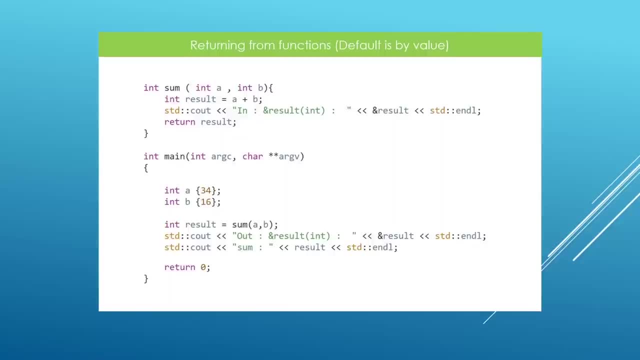 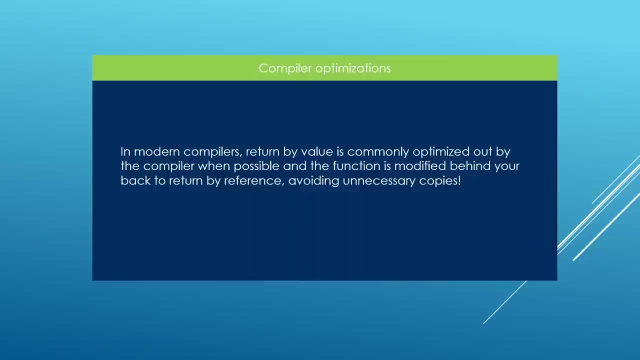 the main function. but things don't always work like this. sometimes the compiler is going to insert optimizations and not really return by value. but returning by value is the default. but if the compiler notices that it can do things better, it is going to optimize your returns by. 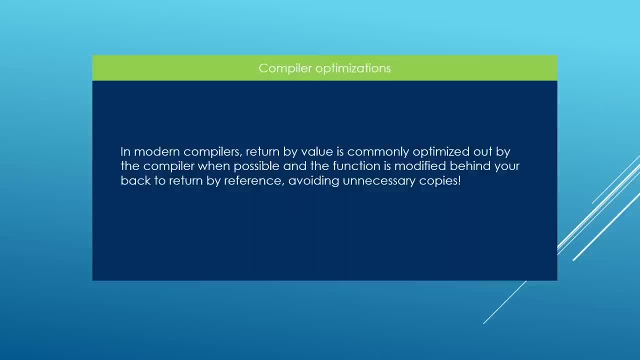 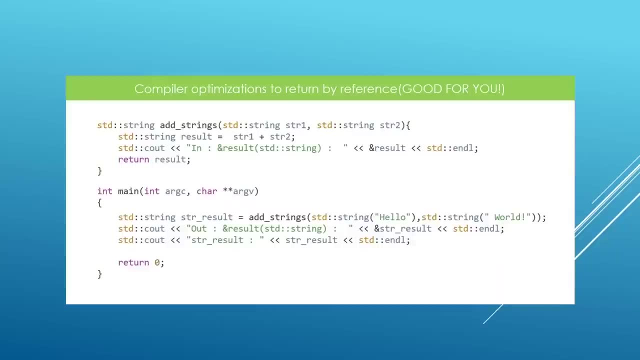 value to return by reference and you're not going to make a copy, but you're going to somehow reuse the local variable in the main function. let's look at a simple example to really drive this home. we have a function here which is going to add strengths. it is going to basically concatenate them using the. 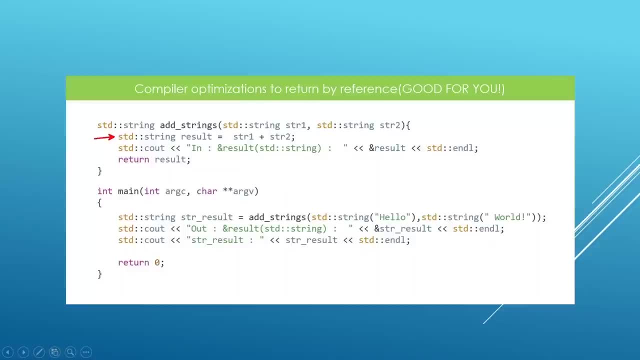 plus operator here. and you notice that inside the function here we're going to set up a local variable which is going to store our concatenated string here and we're going to print the address of the local strength. after that we're going to return the strength so that it 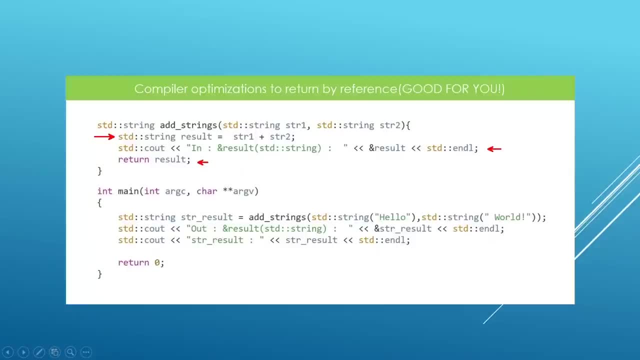 is usable by whoever called this function. let's go in main and see how we can use this function. here we are setting up a variable called str result, which is going to store our result, strength. we are saying add strings. here we are calling our function and we are passing in two strings: hello and world. 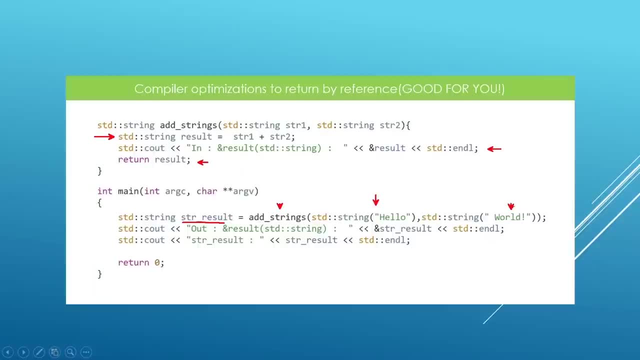 and we want to concatenate these guys. this is going to give us our result and if we're printed out, we're going to get a hello world printed out. but the main message here is that the address of the outside string here is going to be the same as the address we have on the 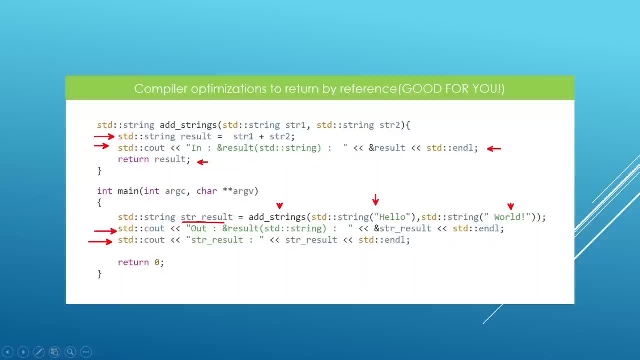 inside here, and this is going to mean that the compiler has actually done some magic to return the local variable because it has seen that we could really be wasting this guy here inside the function. when the function returns this string, result here is going to die off, but the compiler knows that we can reuse that and avoid the work of copying this string, which. 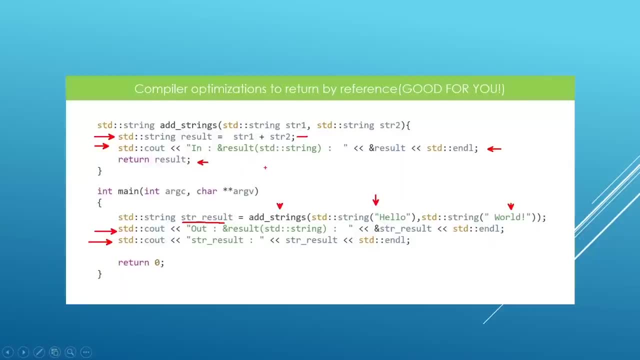 might be really large. suppose this string has a thousand characters inside and copying it would be a waste. so the compiler is not going to return by value, which is the default. it is going to do some kind of return by reference. but it's really not a return by reference because this is a local. 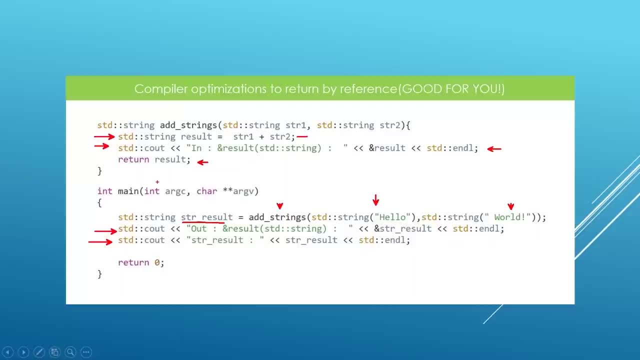 variable. we can't really have a reference to a local variable, to a function. that would be bad because we might be able to modify it when the variable is actually dead, after the function has returned. so it is some magic that the compiler is doing to save you from unnecessary copies. but 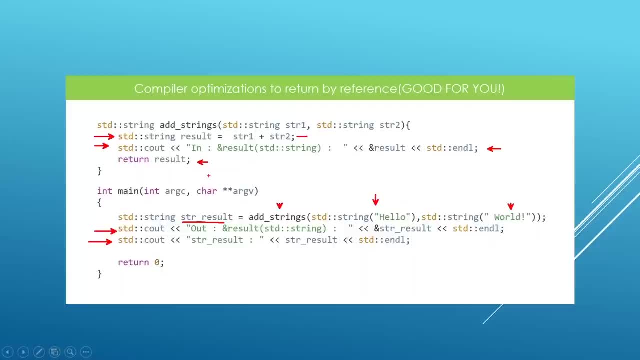 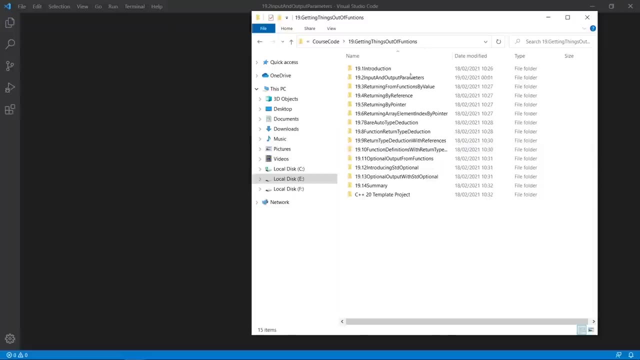 you should be aware of this and not make your code rely on returning by value. okay, now that we know this, we're going to head over to Visual Studio code and actually play with us. here we are in our working folder. the current project is returning from functions by value. 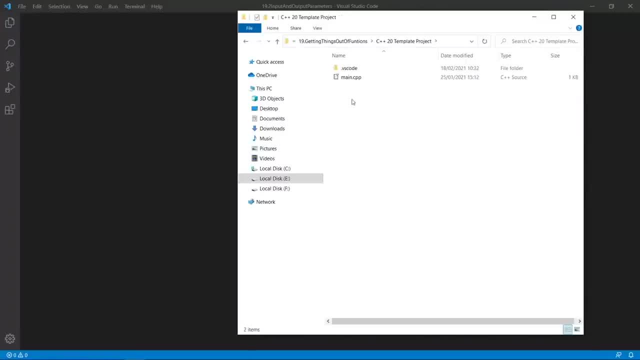 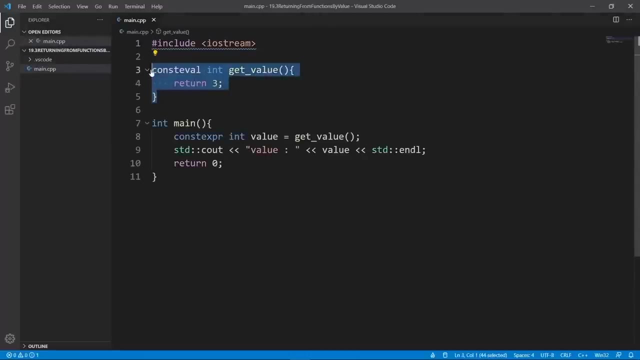 we're going to grab our template files pretty quick. we're going to copy them- let's do that- and we're going to put them in the current lecture or project. and we're going to open this guy up in Visual Studio code pretty quick, let's do that. now we have our main cpp file here we can clean. 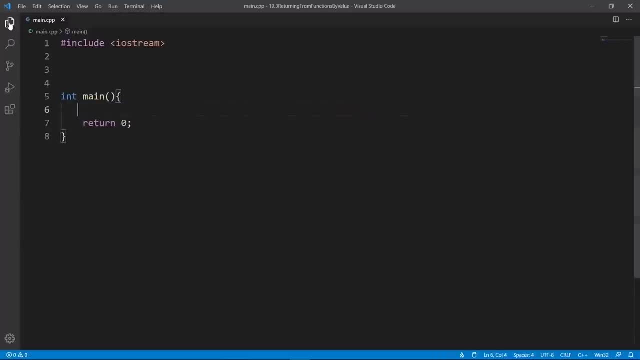 it up a little bit and close the left pane here, because we don't need it. the first thing we're going to do is to put in our function, which is going to compute the sum of two integers and plus the sum of these two guys. inside the function we're going to set up a result variable which is: 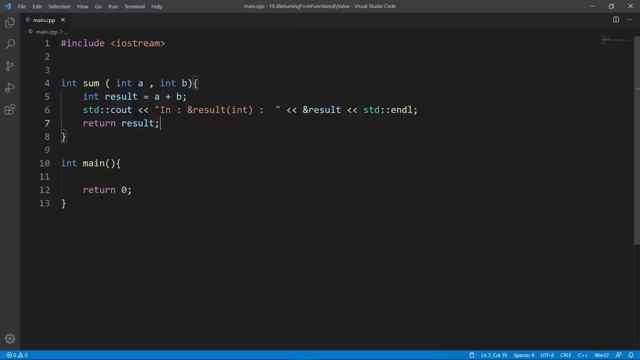 going to store the sum and we're going to return it and it is going to be visible to whoever has called this function. here again, I am going to emphasize that this is going to return by value, so what we return is really going to be a copy of this variable here, and we're going to prove. 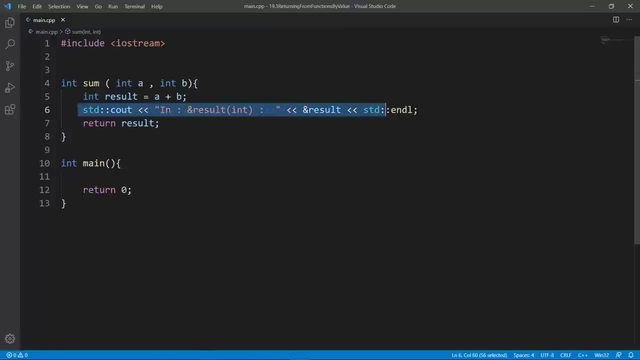 that by printing the address of this variable inside and outside the function here. so we're going to set up two variables in main. we're going to say and X, let's call our input parameters X and Y. we're going to put in a five and the second guy is going to be a Y and it's going to store and a nine. why? 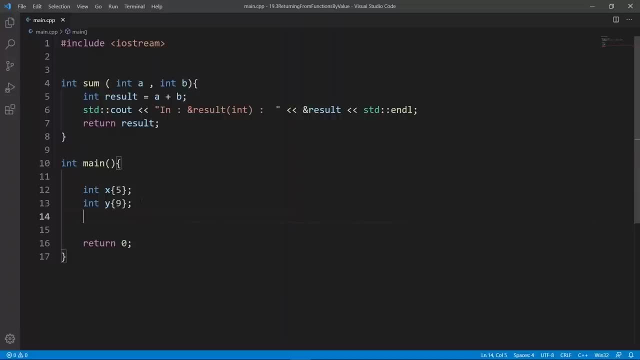 not. after that, we're going to set up a variable which is going to store the results- let's call this result, why not? and we're going to say some X and Y. okay, we are passing these guys by value because we don't really care about copying an ant. it is a fundamental type. it is really small. 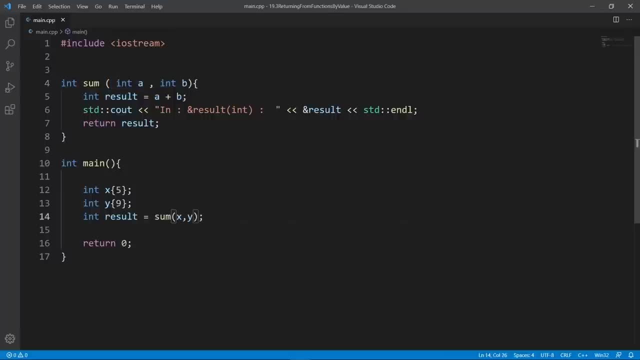 memory. so it's going to be very cheap to copy, it's not going to hurt the performance of our application. but what we want to do now is to print the address of the reserved variable in the main function here and see that it is the same as the address of the variable we have inside here. another 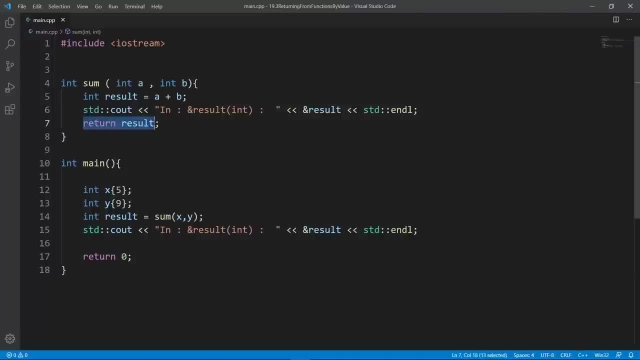 thing you should watch out for is that we are able to get data outside the function. here the sum was a little, but we are able to get it out of the function through the return mechanism here. okay, before we go ahead and run this program, we're going to fix the statement here. we forgot to. 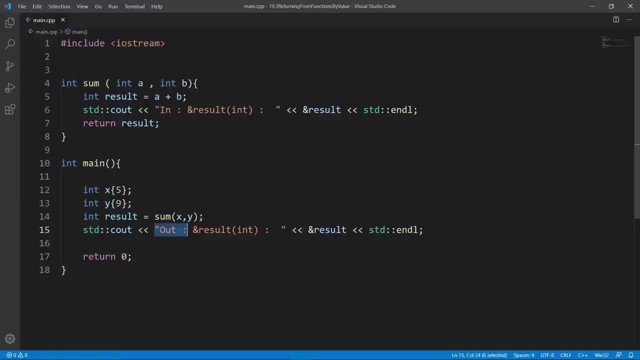 change this to say out to mean that it is outside the function here. that's the meaning. we're going to build with GCC. the build is good, we can clear and run rooster. now we're going to see that inside of the function the address of the result variable here. 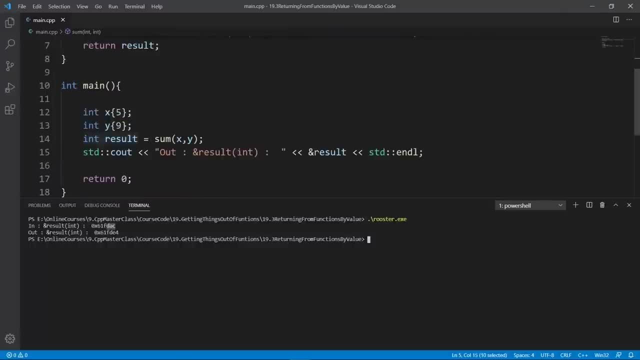 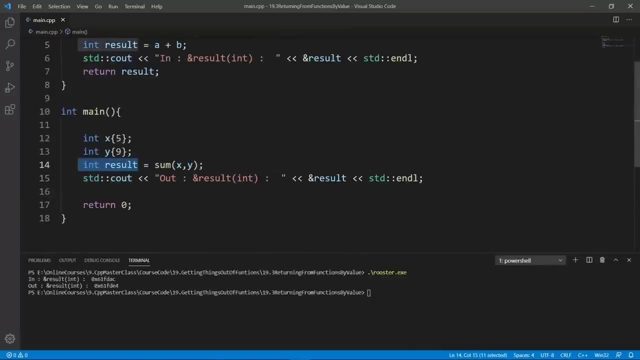 and in DAC and outside the function. when we hit the end of the function here we're going to see that the address ends in de4. so this proves that the local variable inside the function and the outside variable here in the main function live in two different memory addresses. they are two. 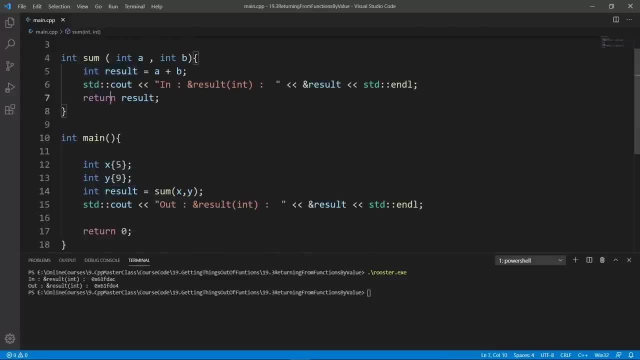 different variables, and the return mechanism here is just going to copy whatever we have in the local variable and make it available on the outside here so that we can assign it to the reserved variable in our main function here. this is how the return mechanism is working and it is going to be returning by value. 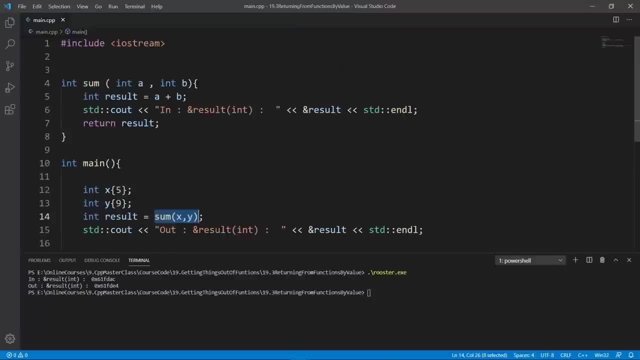 by default, it is going to be making copies. this is the message here. now that we know this, I want to show you that there are exceptions to that rule. if you return by value like this, you won't be really always using separate memory addresses for the inside and the. 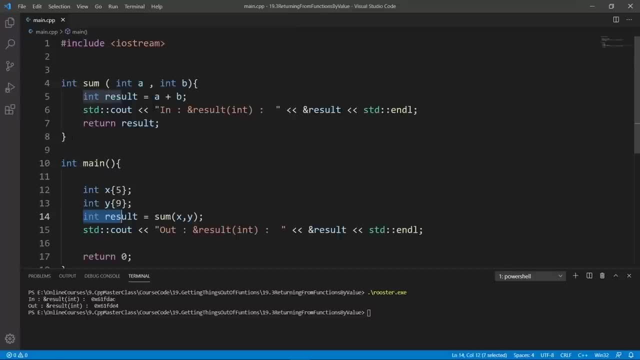 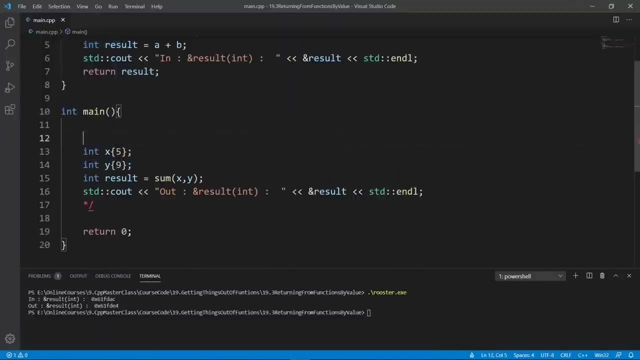 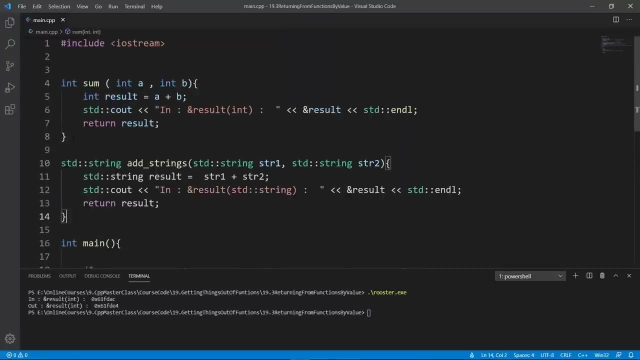 outside here and we're going to prove that with a function that is going to add up two strengths. let's comment what we have out because we don't want this to confuse us. so we're going to bring this inside our block comment here and we are going to go below our sum function here and set. 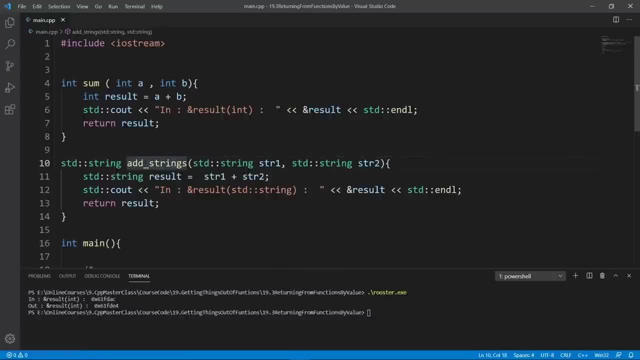 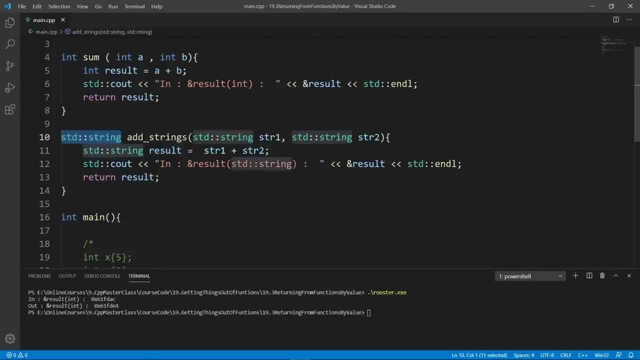 up a new function which is going to be called add strengths. it is going to return a string by value. okay, it is by value, because this return type here is not qualified with anything like a pointer or a reference. so by default it is going to be by value and inside, you see, we are doing the exact same. 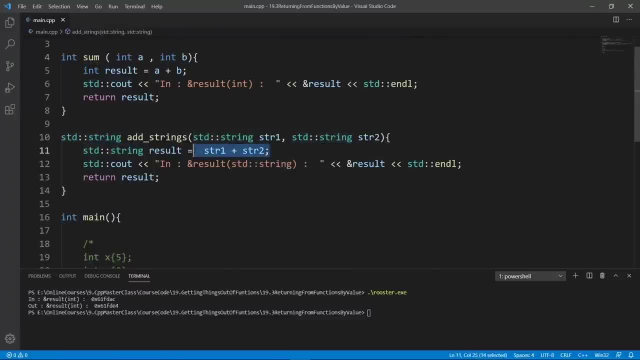 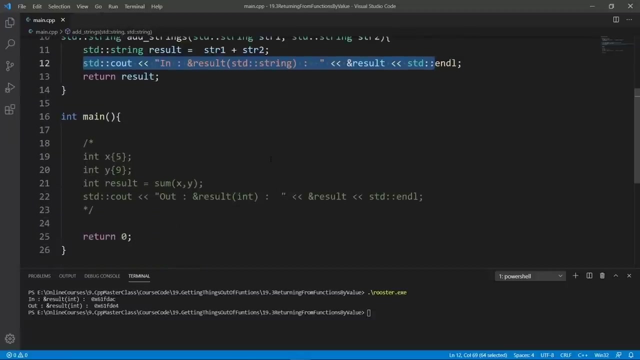 thing we did in the sum function. here we are adding up two strands, we are storing the result in a local variable and we are returning that. but if we run this program you're going to see that the address on the inside is going to be the same as the address on the outside. so let's set up 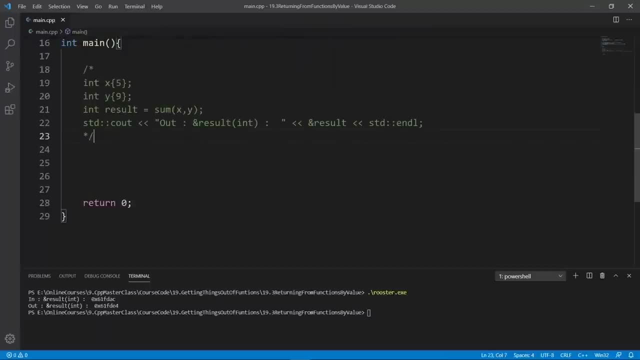 something that we can play with here. we're going to go down in the main function and set up a few variables. we're going to say hdd strength, we're going to say n, str1, and we're going to store in hello, let's do that. and we're going to say std, strain and str2 and we're going to 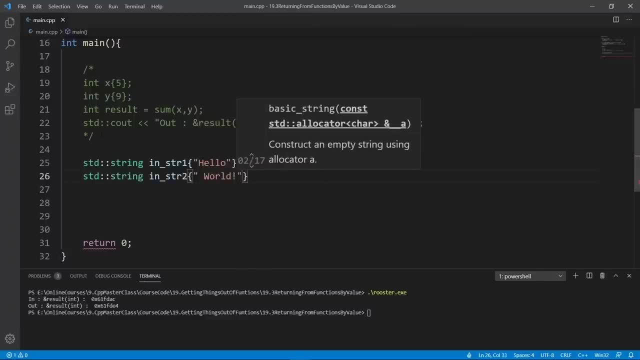 store n world by now. you know what I am trying to do here. I am trying to say hello world. okay, once we have this, we're going to set up a result Stern. so we're going to say std strength and let's say result str, and we're going to say add str and we're going 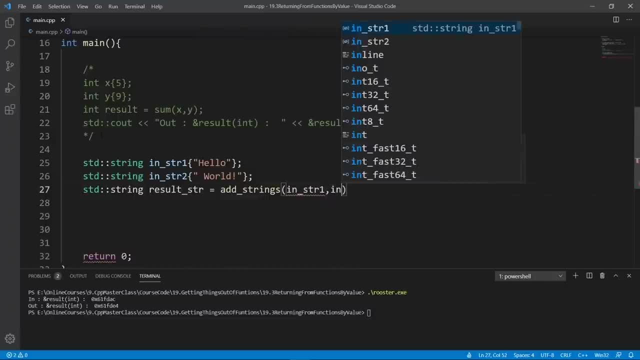 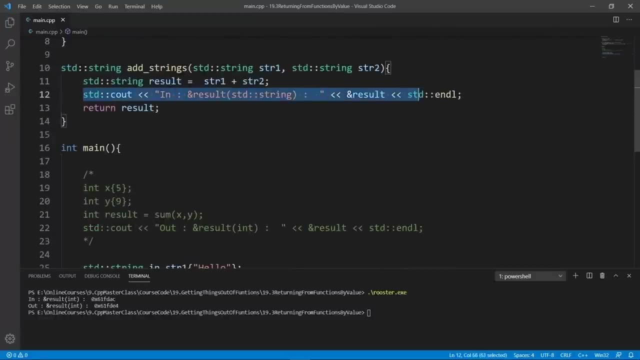 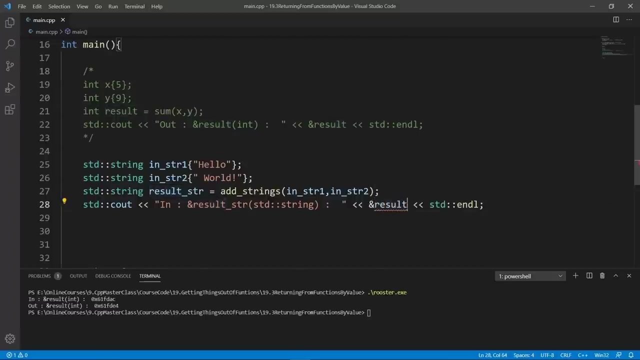 up in str1 and in str2. this is how we do this, and after we do this, we're going to print out the address of the variable here, so let's do that. and it is going to be the address of result str. let's say that here. and we also need to print the actual result of this operation here, so let's do. 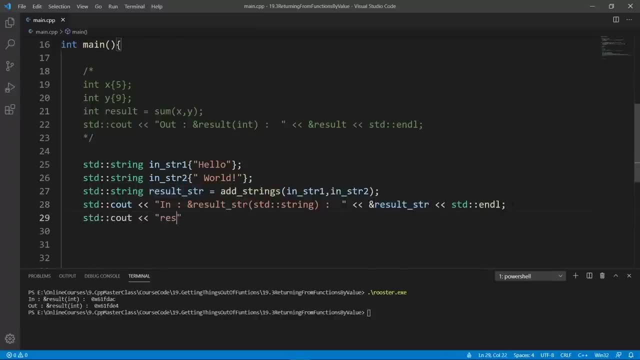 that we're going to say sdc out result str. we're going to print the actual strength. i don't think we did that on our sum function here, but we can quickly go there and prove that to you. so let's comment this out. sorry for this, this is going to be confusing, but i don't want to leave you with. 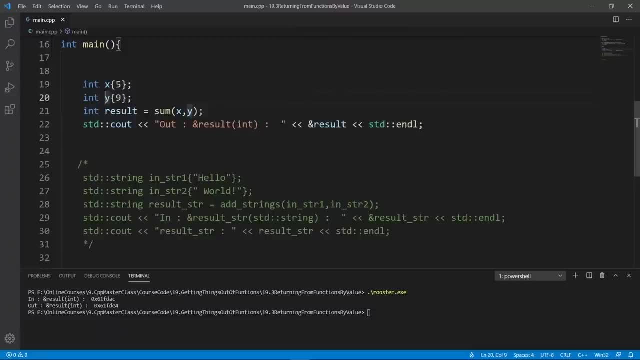 unexplained things. so we're going to see that if we print this out, we're going to get the sum, which is 14, printed out. let's do that pretty quick. we're going to go down and say stdcl and say result and we're going to say: 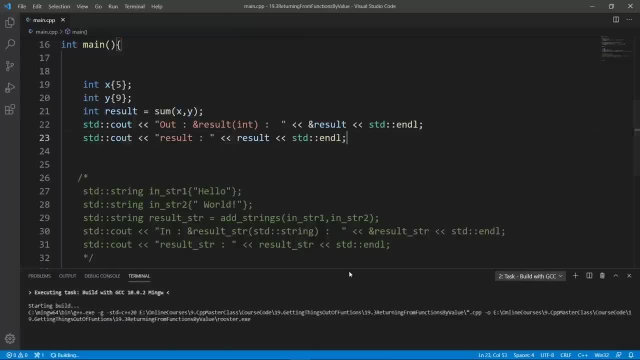 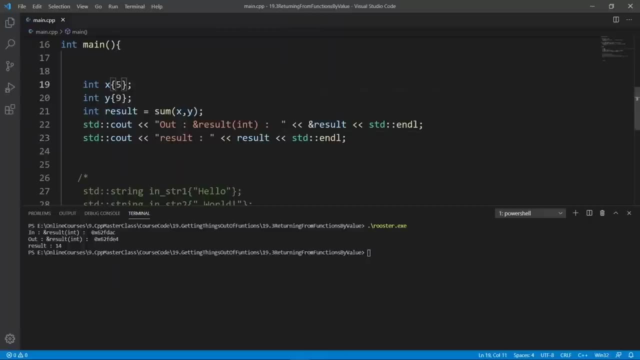 result and we're going to build pretty quick with gcc and if we clear and run rooster, we're going to see the result which is 14 here and you can change these guys up to really play with us. for example, if we make this 15 and put in a 9, we're going to get a 24 printed out. let's build. 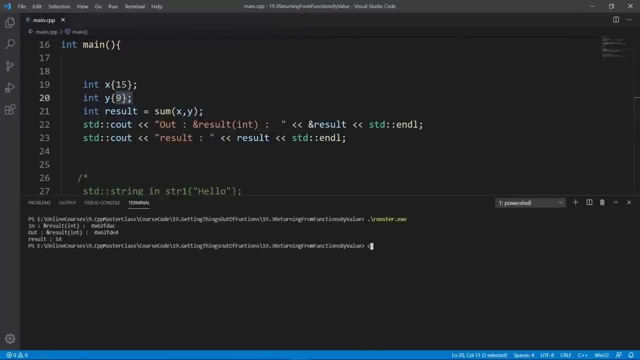 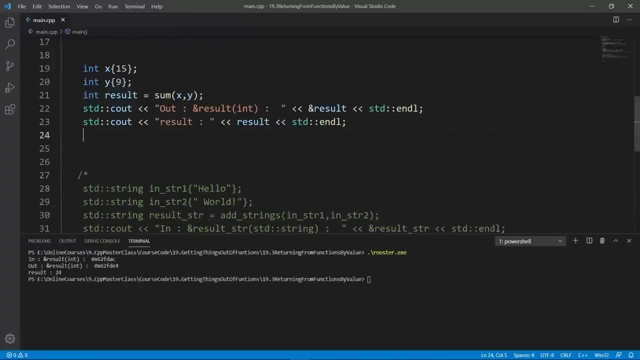 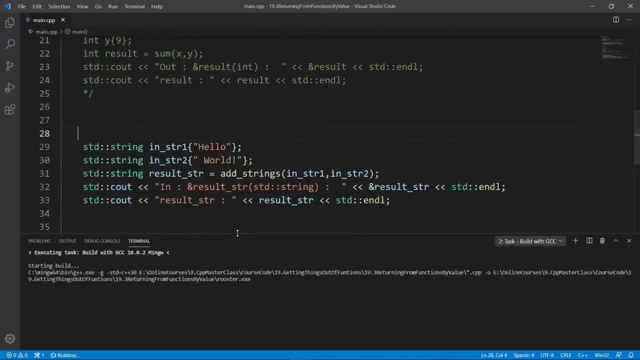 again just to have fun with this, and we're going to clear and run rooster. we're going to get a 24 here. now we can comment this back. i am happy i have showed you this and we can uncomment our string code here and, uh, build and run it. so we're going to build with gcc. the build is good, we can. 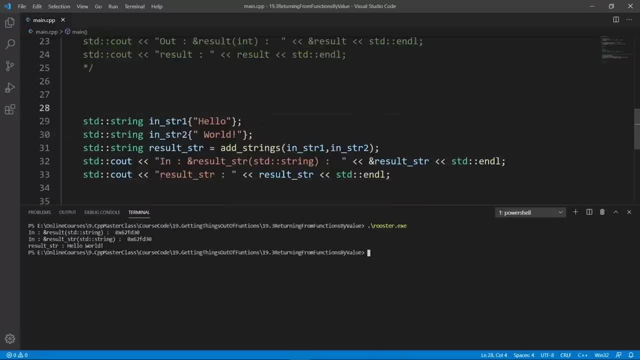 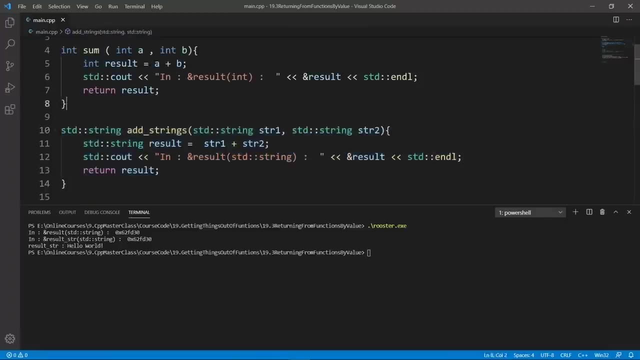 clear and run rooster. and again, what we want to see is that the compiler is going to optimize this out. it is not going to return by value, like we had with the sum function, where we had the address on the inside different from the address on the inside of the address. on the inside of the address. 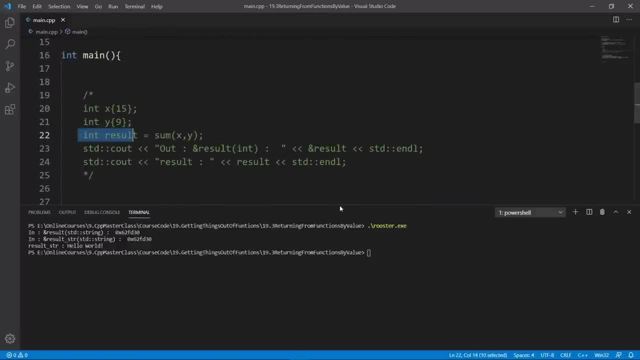 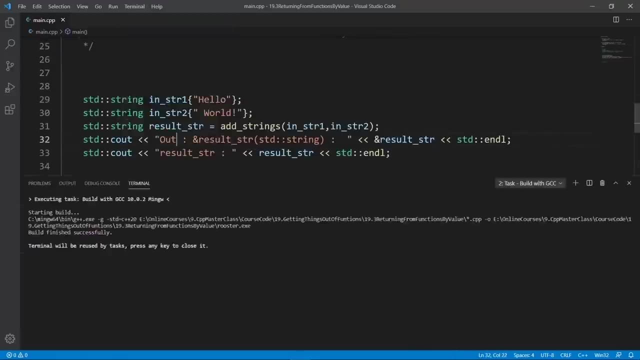 the outside. you see here that inside, ah, we forgot again to change this guy to out. sorry for this. so we're going to make this guy out and we're going to build again and we're going to clear, clear and run rooster. now we're going to see that inside the address ends in d30 and outside the address ends. 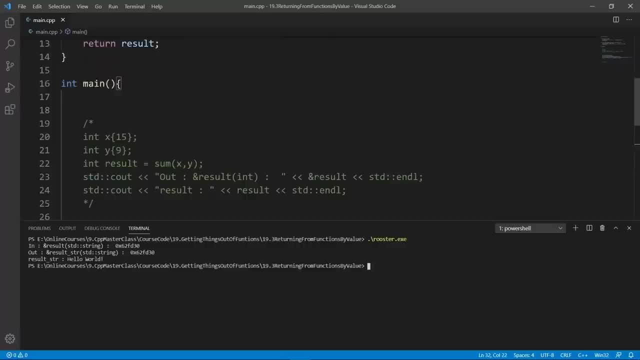 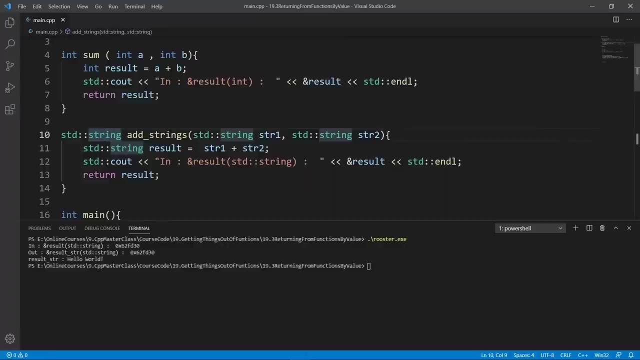 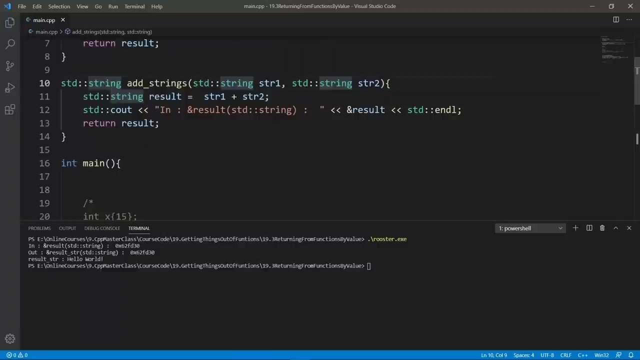 in d30. this can be really confusing because we said we wanted to return by value by not decorating up any of the values that we just made. so if we make a copy of the address now inside the inside, the inside and the address on the inside should be different, but they are the same. the reason is. 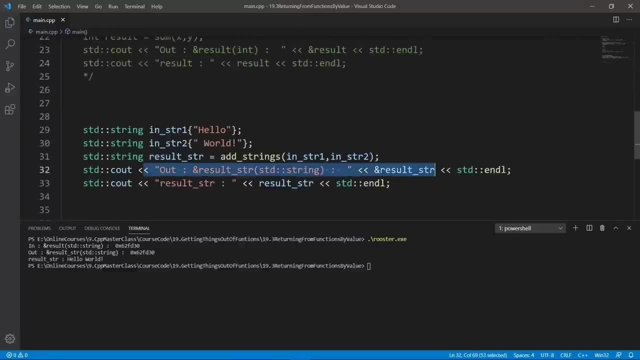 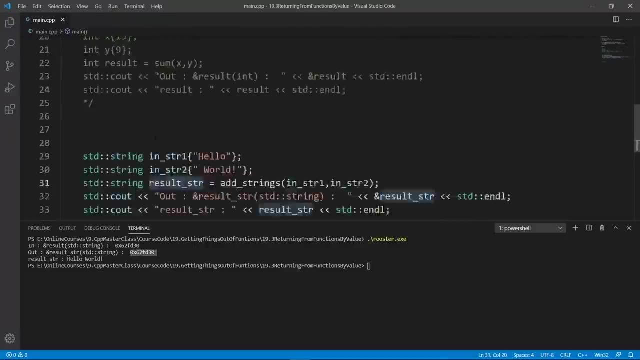 the compiler is going to notice that you are trying to copy strings and it is going to see that the variable here, which is inside the function, is going to be wasted when the function returns by default. this is what it actually does, so it will go to the function by default and when 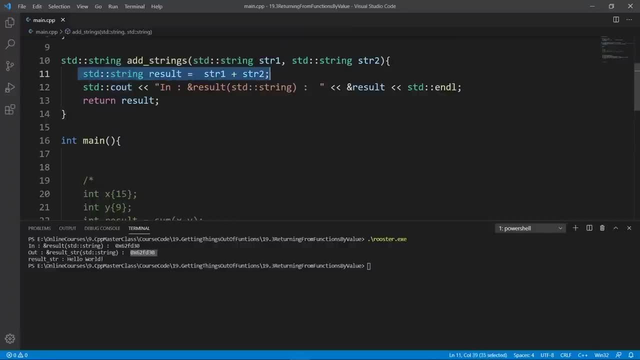 it returns, you click ok and that's it, and then, when it returns, it goes on the code, which is an fault. this should be really destroyed and you should copy, because you are returning by value, but the compiler is going to insert an optimization to do some magic and make it look like you are. 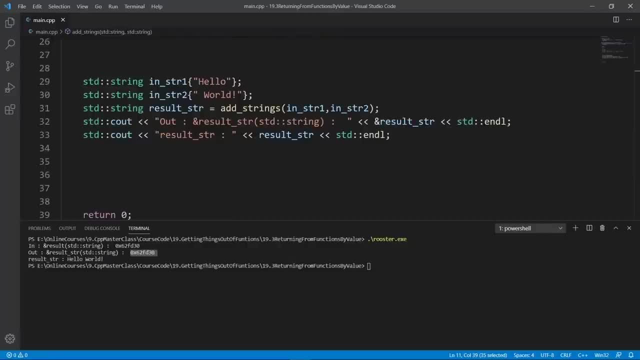 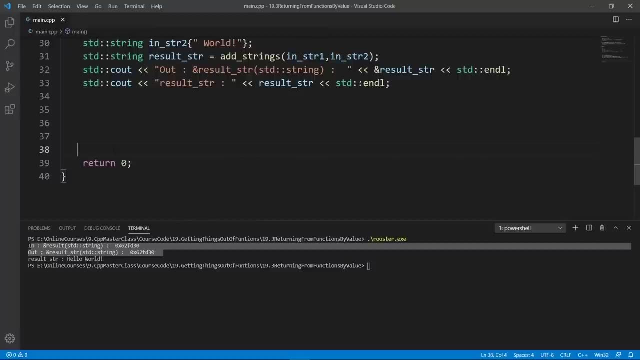 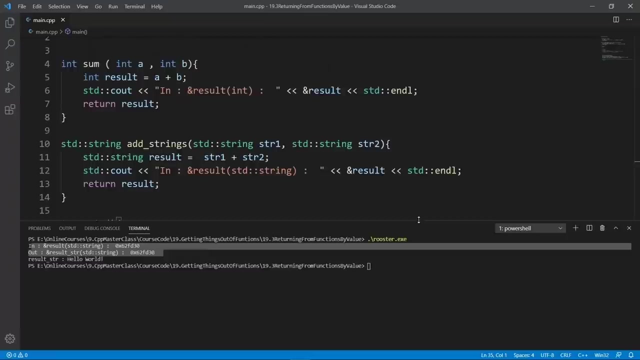 returning by reference and it is really not going to make a copy, so it is going to reuse the address on the inside and hopefully this is going to prove this to you. the message here is that you shouldn't rely on your functions returning by value, because if the compiler sees that, it can do a better job. 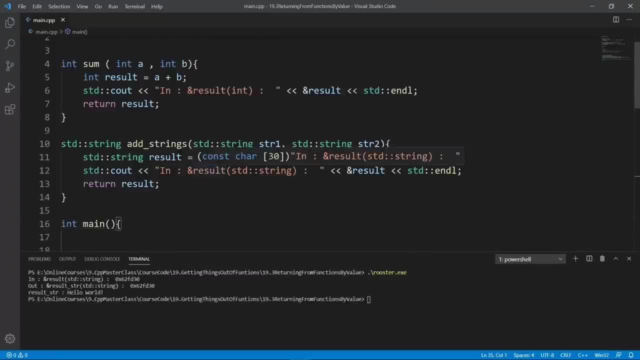 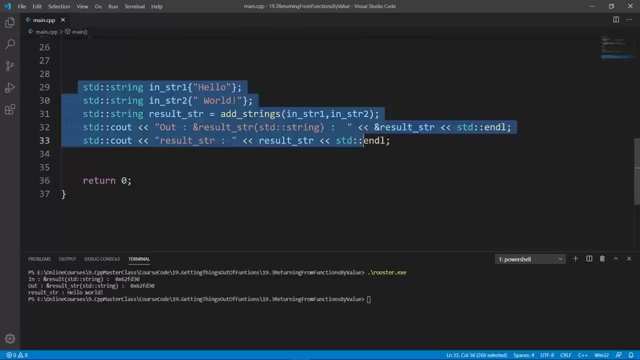 than you. it is going to optimize your return by value to return by reference and you're going to not be making copies, so don't make your code rely on returning by value and making copies, and you should be aware of these optimizations that the compiler can do behind your back. i would like to 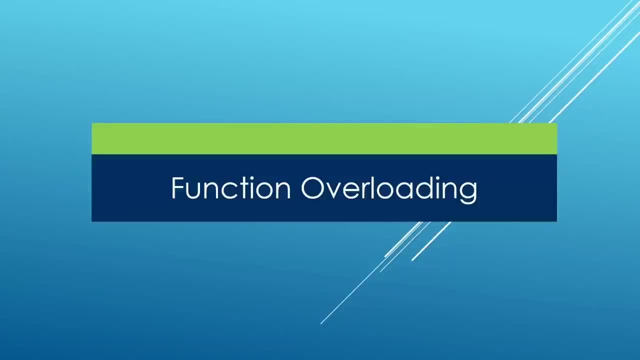 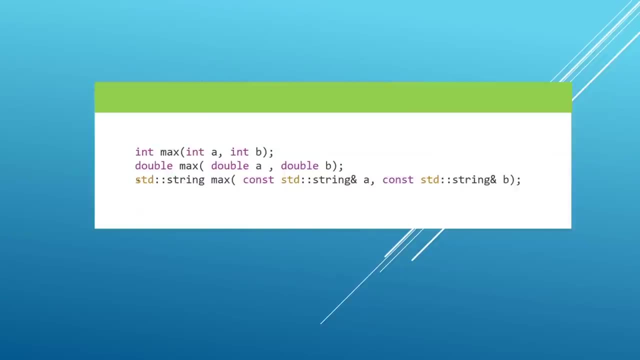 welcome you. new chapter where we will be learning about function overloading. function overloading is a mechanism we have in c++ to have multiple copies of the same function, but taking different parameters, for example. here you see that we have different functions but all these functions have. 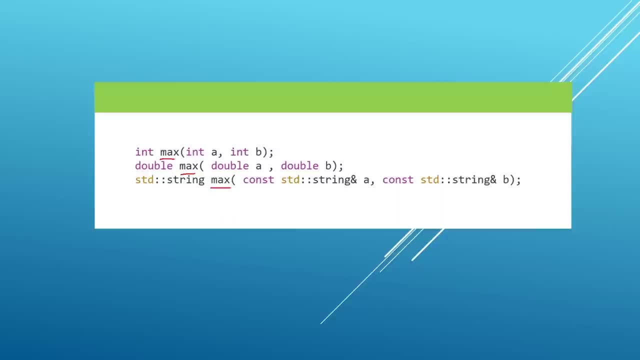 the same function name, and these are said to be different overloads of the same function. there are a couple of rules you need to be aware of to be able to set up your overalls correctly and get them to work, and that's what we're going to be learning about. 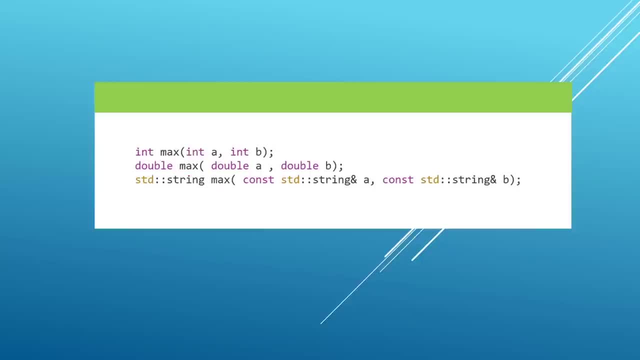 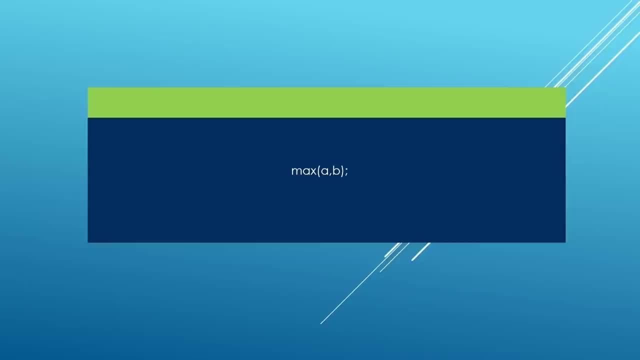 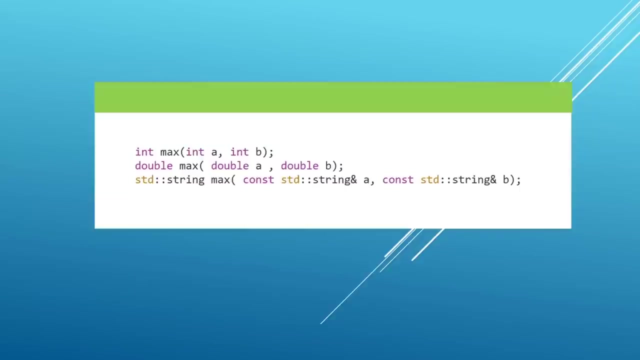 in detail in this chapter. but now i just want you to see the flexibility you can get with function overloading, for example. here, if we have a few variables in our program, we can call the max function and the compiler is going to select the most fitting overloading here. so for example, if 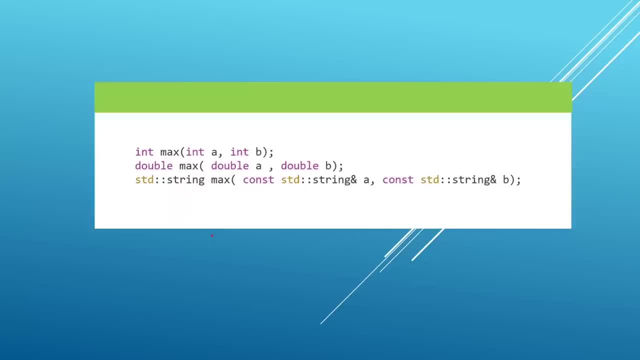 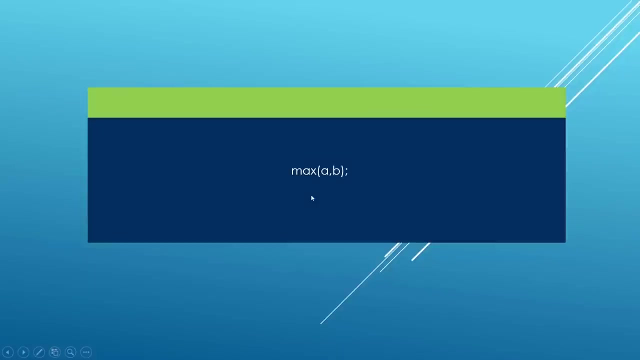 we call our function with integer arguments, the compiler is going to choose this overload here. and if we call our function with std string arguments, the compiler is going to choose this overload here and we don't really need to concern ourselves with making sure we have the correct arguments. 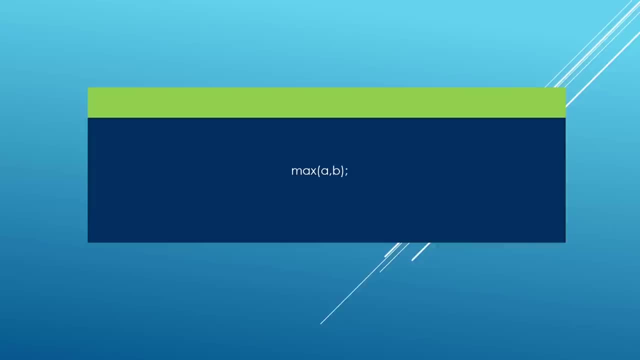 the compiler is going to choose the correct function overload for us and it is going to call it, and it's going to be very flexible to call these functions from our c++ code. this is how function overload can be really useful. we are going to stop here in this lecture and the next. 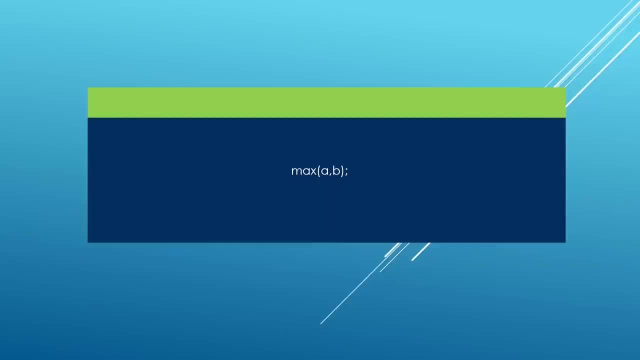 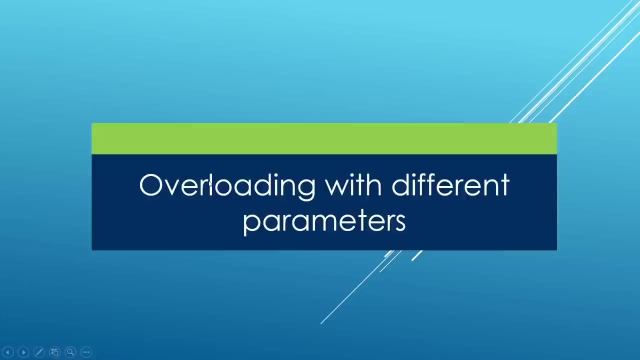 one we're going to learn about how you can set up function overloads based on different function parameters. go ahead and finish up here and meet me there. in this lecture, we're going to see how we can overload functions based on the parameters that we pass to the function when we are declaring. 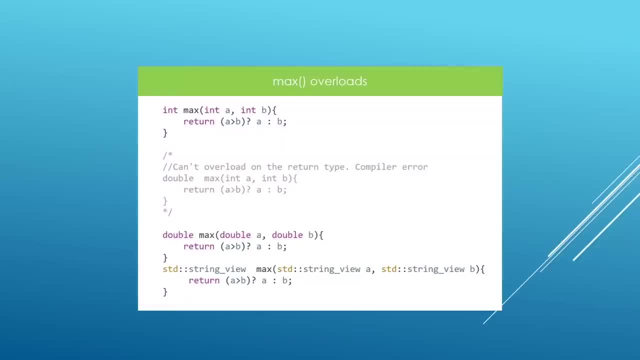 it or defining it. and here is a simple example to drive the point home. here we have a function called max, and this is the name. it is taking two parameters which are of type, and here, and by overloading this function, we will have to use the same name. 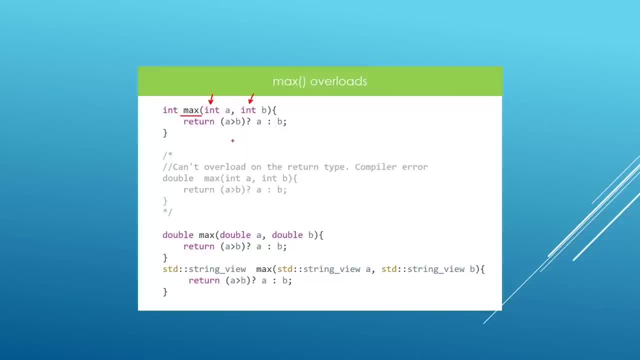 as this function here. so the differences really will be in the parameters that we pass to the function, because the return type isn't involved in defining the signature of the function. so if we try to set up another function called max here, which takes the exact same parameters as our max, 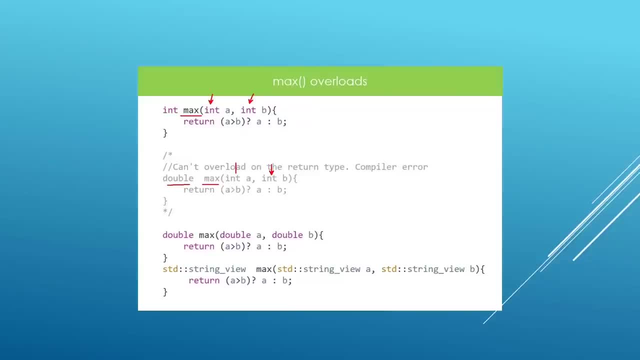 on top here. the difference is only going to be in the return type. the compiler is not going to allow us to do this, because the return type isn't really significant in making two functions different. okay, the only way we have to set up a function which is legal in c++ is to change something about. 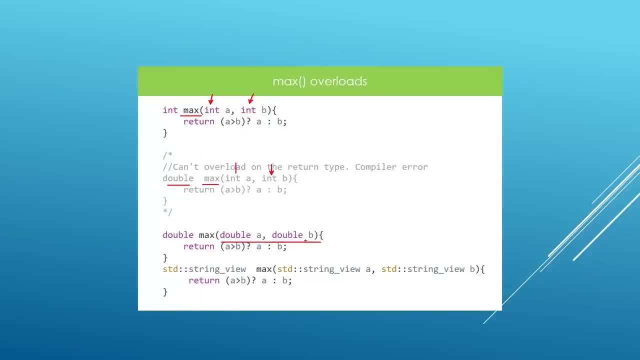 the parameters that we have here. we can change the types, like you see. here, for example, we change the types to b double. if the types are different, we might even change the order of the parameters. you just have to make sure the parameter list is different in one way or another. that's how. 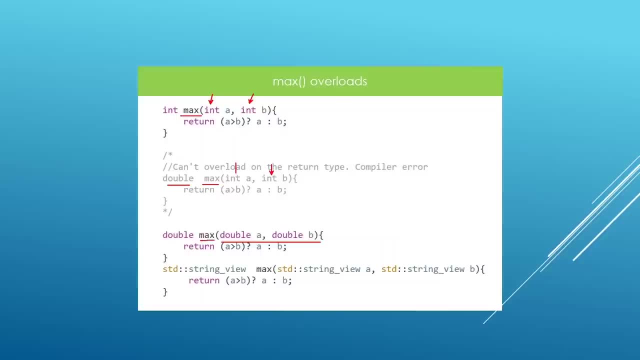 you're going to get this function to run with the same names here and if we manage to set up multiple functions with the same name in c plus plus, these functions are going to be called overloads of each other. okay, if we go down here, we have another overload for the max function. this overload is: 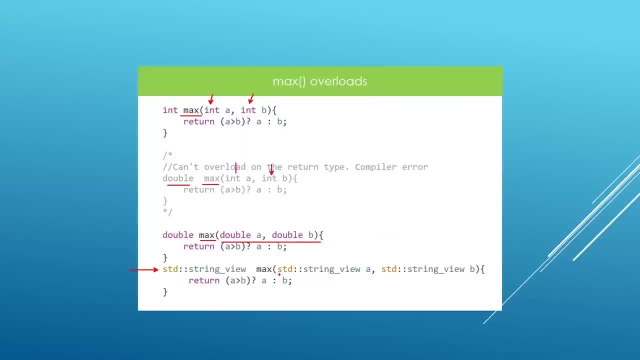 going to take two parameters, and the parameters are going to be of type string view. they are different from stick. std string view are going to be of type string view. they are different from multiplicating rajad heyy, what we have on top here, which is ant, so this is a legal overload for this max function here. 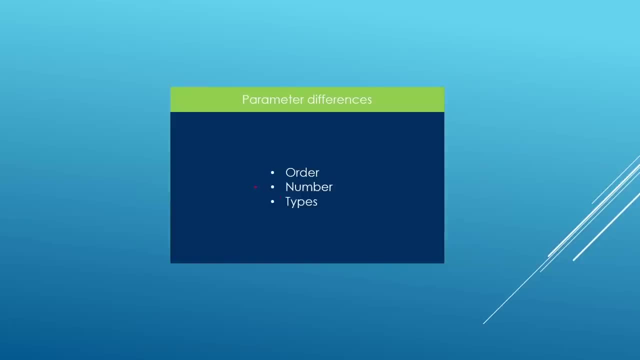 and we can use it. okay, we really have a few ways we can make our function overloads by now. we can change the order of the parameter, we can change the number of the parameters or even we can change the types of the parameters. again, function overloads are a mechanism we have in. 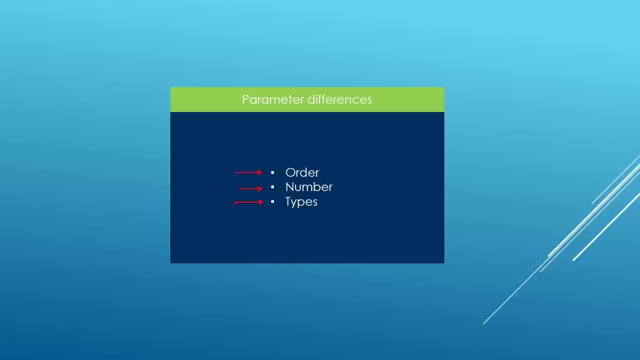 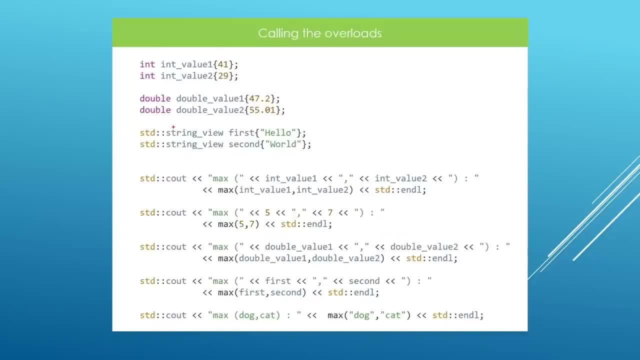 c plus plus to set up multiple functions with the same name to make our code easier to work with. okay, now that you know that, let's look at a simple example of how we can call our overloads. we have a few variables declared here. we have int variables, we have double variables and we have std string. 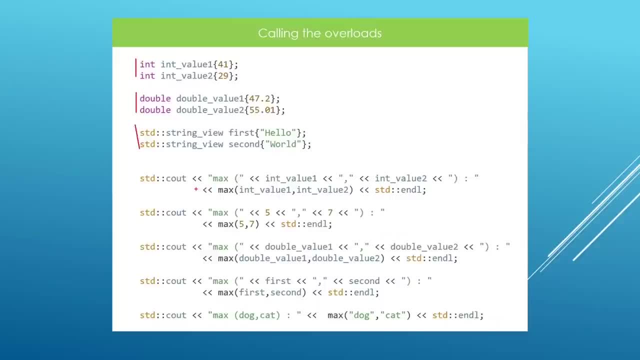 view variables. and if you go down here we are calling our max function passing in integers, so the overload that takes integers for this max function is going to be called here. down here we are passing in integer literals, so this is going to call the int overload. down here we are calling the function with double parameters or arguments, so this is going to call: 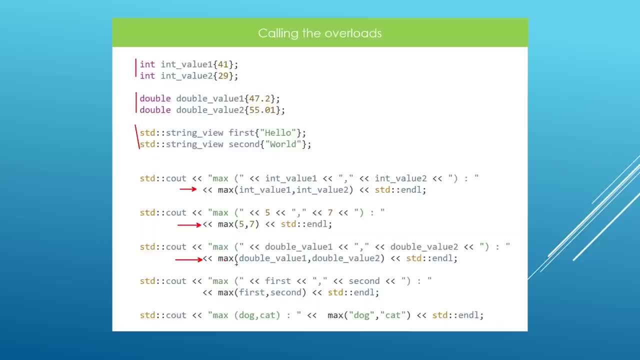 our double overload for the max function here and down. here we are passing in our string view parameters and this is going to call the overload. that takes string view parameters. and the last guy here is going to take two string literals. string literals is going to take two string literals. 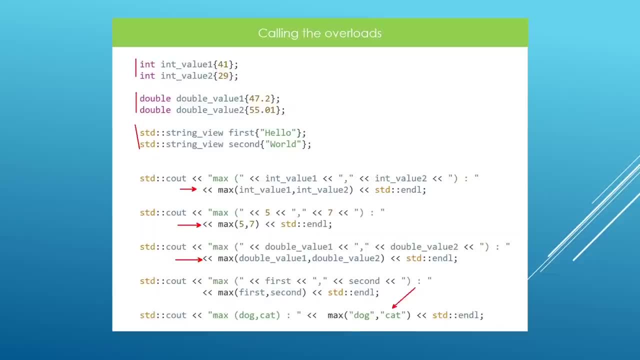 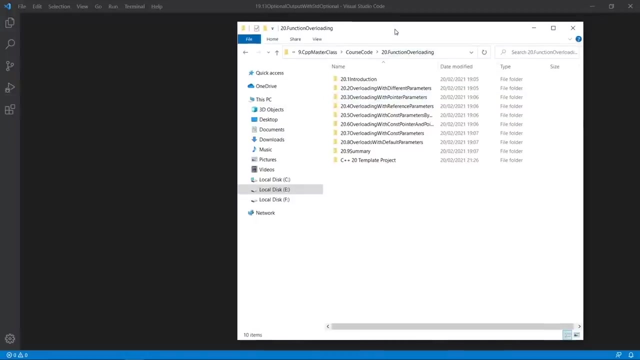 can implicitly convert to std string view, so our std string view overload for the max function here is going to be called. now that we know this, we're going to head over to visual studio code and play with this a little more. okay, here we are in our working folder. the current project is: 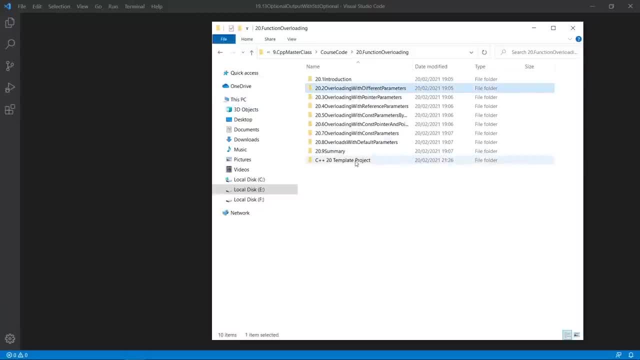 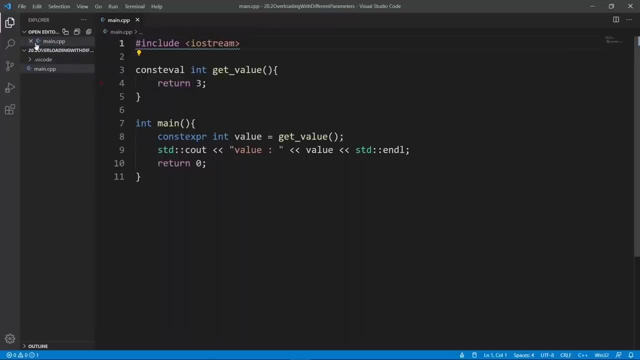 overloading with different parameters. here we're going to grab our template files, like we always do. we're going to put them in place and we are going to open this guy in visual studio code by dragging and dropping on top of visual studio code. here this is going to open our project. here we're going to click on our main cpp file. 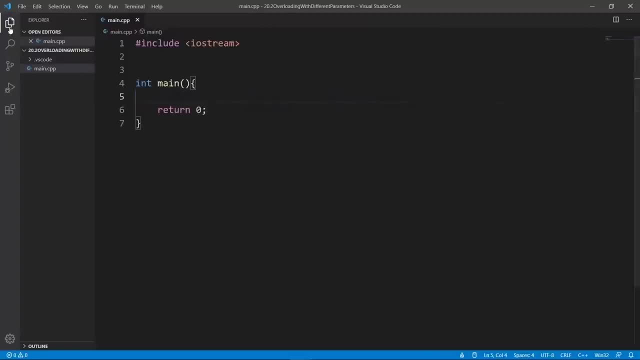 and open it. we're going to clean it up a little bit and close the left pane here. we are going to go on top here and put in our first max function. here the return type is end. in this case it is going to take two parameters and it is going to return whichever number is the maximum. 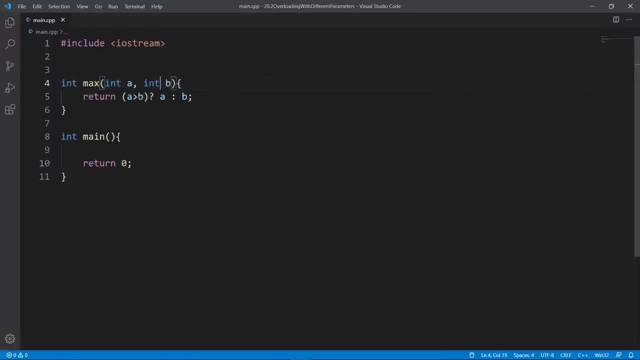 and we are taking parameters in by value and returning by value. here nothing special. we can go in main and call this function, and you already know how to do that. i don't think i really need to do that. but now what we really are interested in is being able to set up different functions. 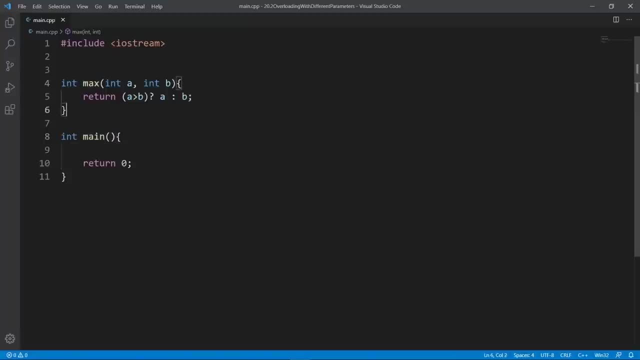 with the same function name, like we have here, because if, for example, you take this function and put that down below, we're going to make a copy of it and only change the return type. if we try to compile this program, you see that even visual studio code is unhappy. now if we bring up 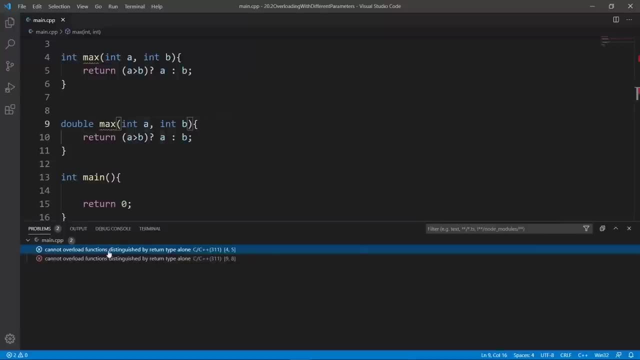 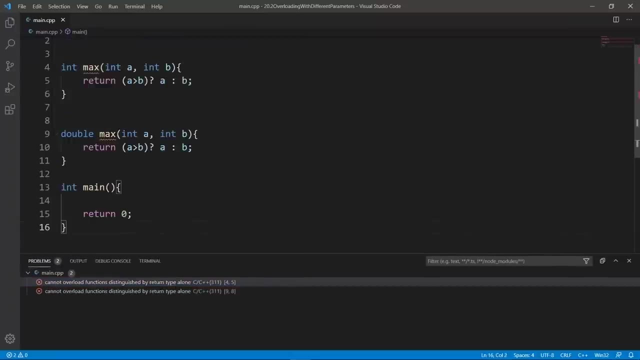 a terminal, it is going to tell us, cannot overload function distinguished by the return type alone. so again, the message is super clear here. the return type is not enough to make two functions different, because the return type isn't involved in making the signature unique. what makes the 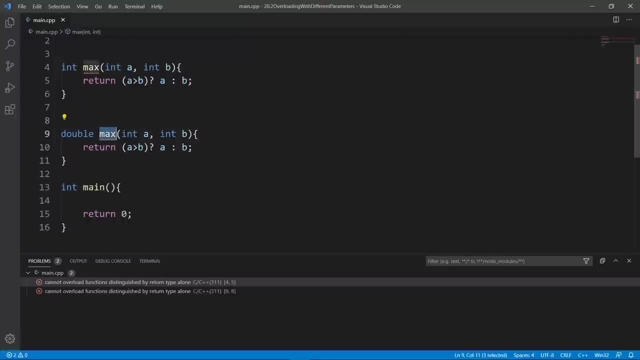 signature. unique is either the function name or the parameters that you pass to the function here. so we're going to make this return type back a double and we're going to figure out a way to make these two functions different but have the same name here, because sometimes you really want this. one way we have to do this is to change the 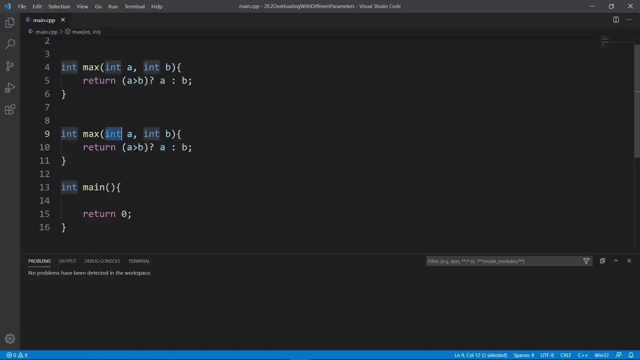 types of the parameters that we pass in here. so we're going to make them double and we're going to make them double here and this is going to be valid c++ code. these two functions are different, even if they have the same name here. they are two different functions because they take different parameters. so if you try to call, 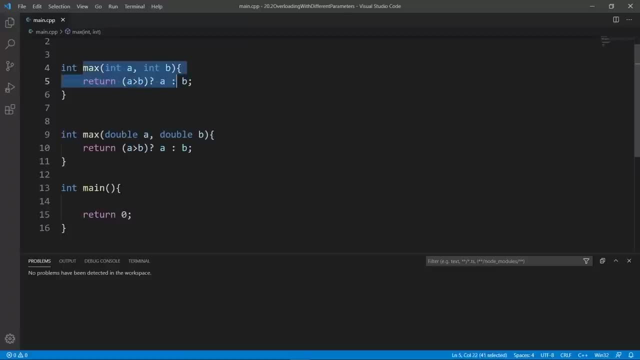 this function with integers. this one is going to be called which takes integers in. if you call it with double arguments, this guy here is going to be called. let's try and prove this. so we're going to go inside and say stdc out and overload called. i think this is enough and we're going to go in. 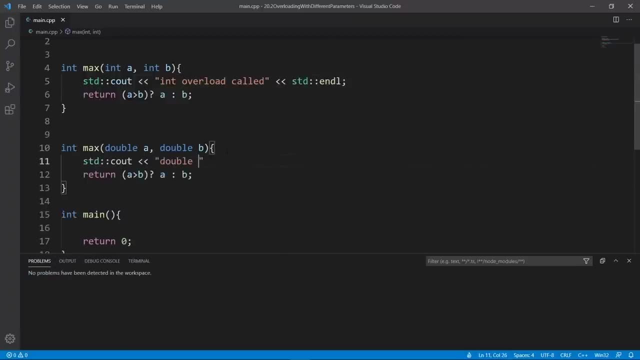 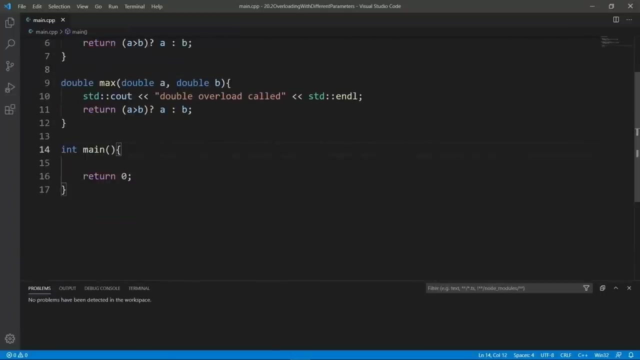 the double function here and say: stdc out, double overload called. okay, once we have this, we also have to change the return type here to double, because it's going to make things a little bit consistent here. but now we want to go in our main function here and set up. 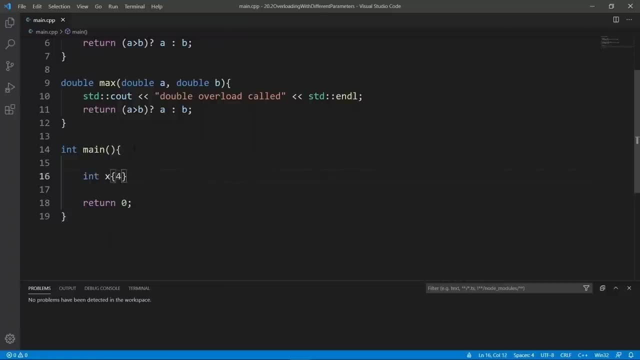 a few variables. we're going to say and x and we're going to make this a four. and we're going to say and y and we're going to make this a nine. why not? we're going to set up also double variables. let's say double a and say five. point four, two. 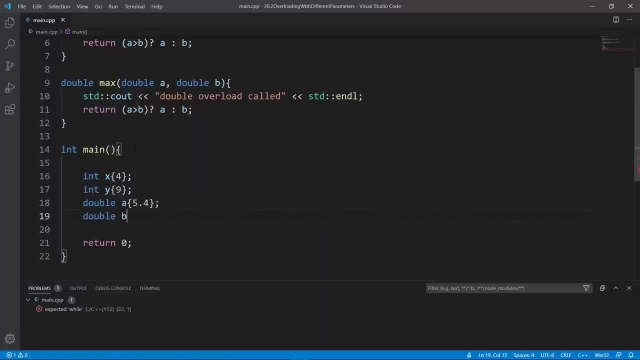 make it a double variable and we're going to say: double b and a, put in 7.4. why not now? we are going to call max, we're going to say auto result and say max and pass in x and y. what do you think we're? 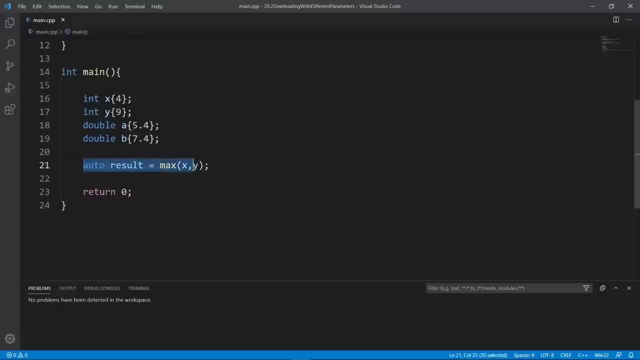 going to return here. so what we really are interested in is the return type of the result variable here and the compiler is going to deduce whatever is returned by this function. if we call the function with x and y, x and y are integers, so the compiler is going to search for a function. 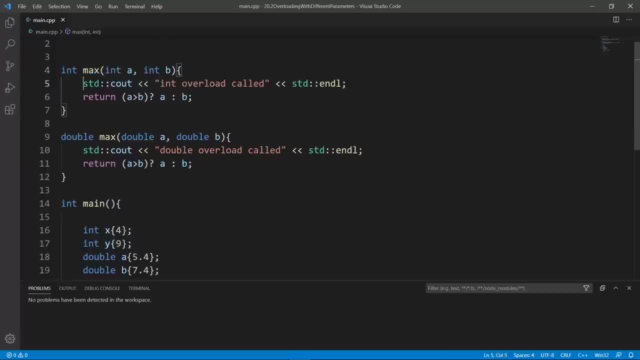 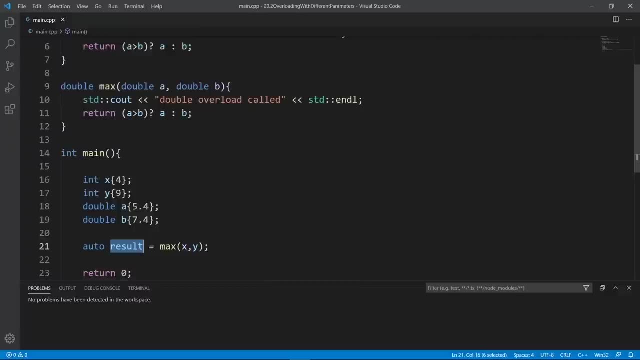 that takes integers and it's going to find this guy here and that's what it's going to be called. let's build and run this program. we are not interested in looking at the output here, we're just going to see this. std out statements here, print whatever function was called. okay, we expect. 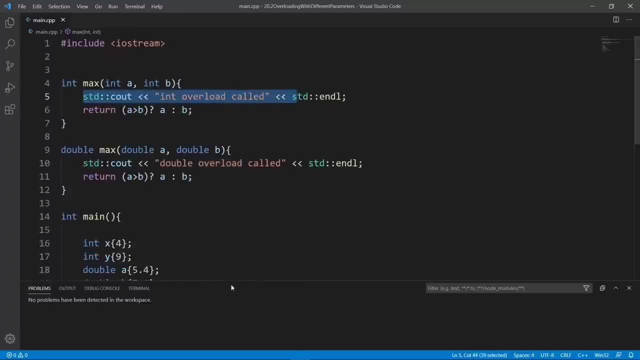 the end one to be called. so we're going to see ant overload called on the terminal here when we run this program. so let's do that. we're going to build with gcc like we always do. the build is good, so we can clear and run rooster. we're going to see int overload called, okay, so this proves that we can. 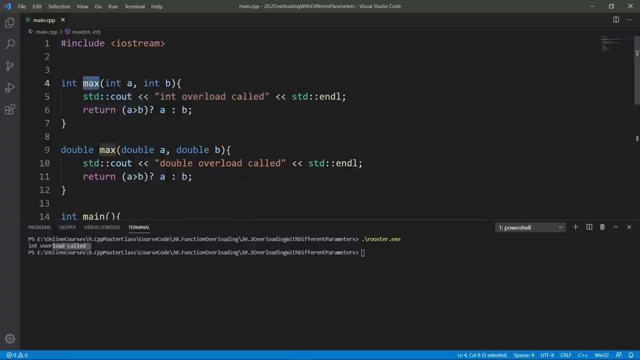 set up two functions with the same name and make them different only in the parameters that they take, and the differences may be either in the types of the parameter, like we are doing here. they may also be in the order of the parameters, and we're going to. 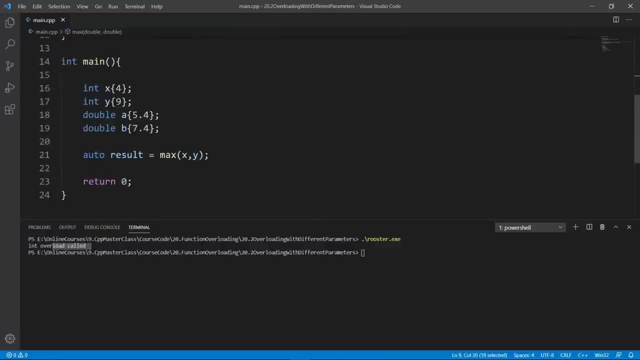 see an example of that in a minute. but before we do that, we also need to try this with a and v and show you that the double one is going to be called because we are passing and double arguments here. so let's build again. the build is good, we can clear and run rooster. this is going to call. 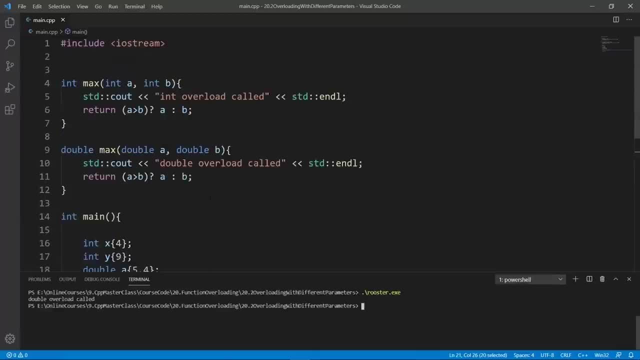 our double overload. hopefully this really drives the point home that we can set up multiple overloads for the same function name and again the differences are going to be in the parameter that we pass. here we have been able to pass different types for the parameters and this was legal c plus plus code. but we can also set up another overload just by changing. 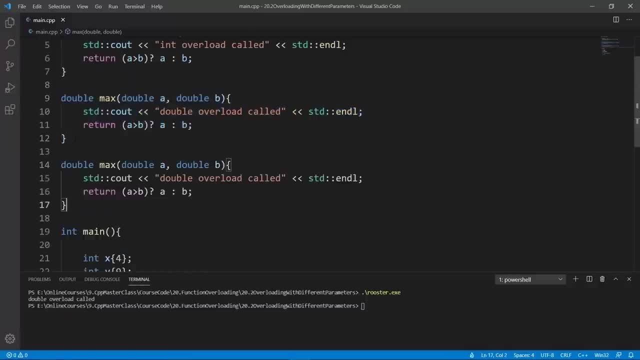 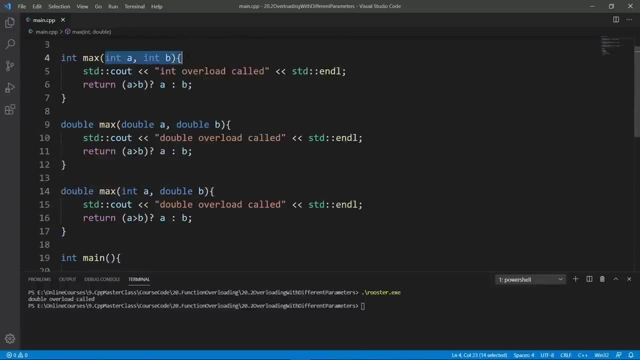 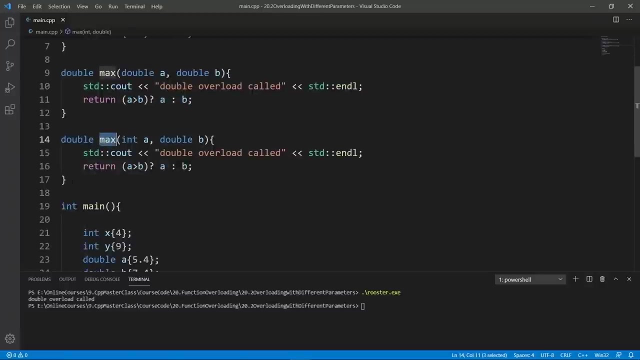 the types and the order of the parameters. let's do that. we're going to make the first parameter here and, and once we do that, this is different from any of the overloads we've had. so this is a valid overload for this max function here. this is going to work. we can even change the 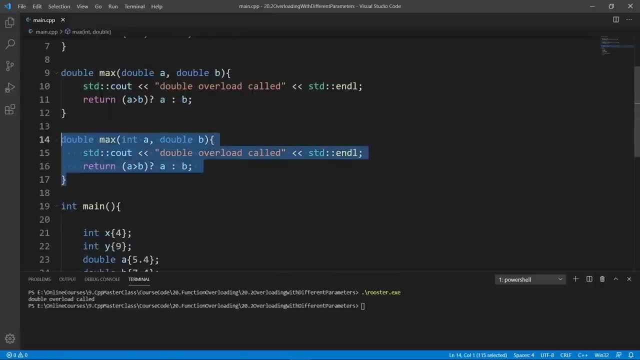 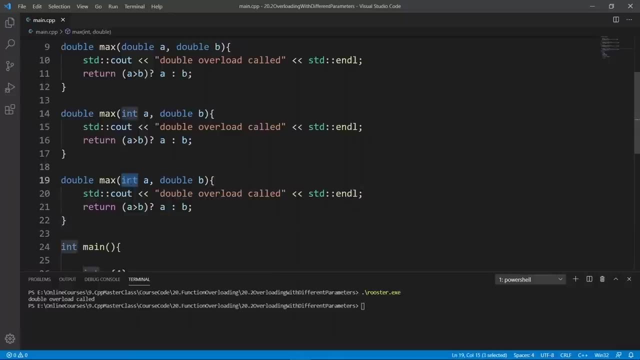 order of these two guys and it is also going to be a valid overload. let's put in another variant of this guy and we're going to change the first parameter to double and the second one to end, and now we have four overloads for the max function and again, the message here is that you 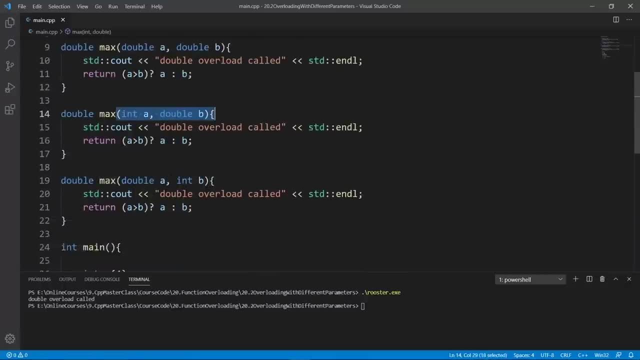 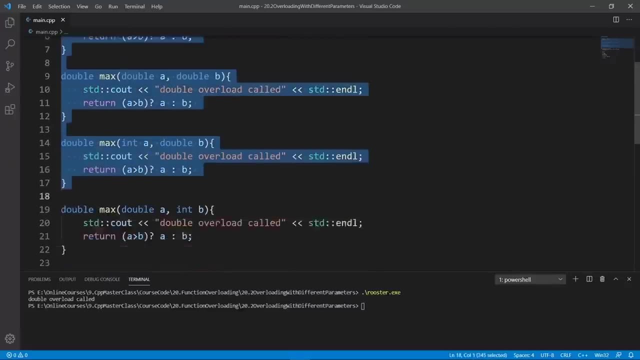 just have to make sure the parameters are different in some way and your overload is going to be valid. and again, i'm not telling you to set up functions like this, because in this case this is really useless, but i am trying to expose this facility to you. 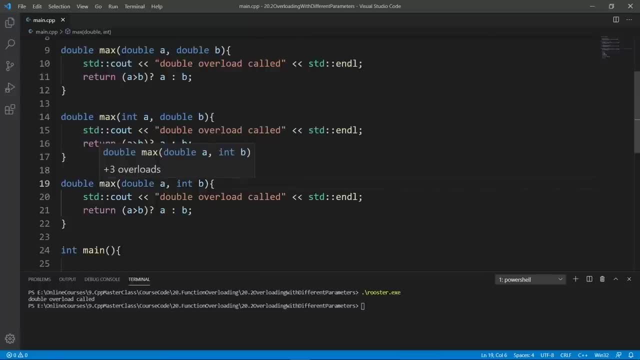 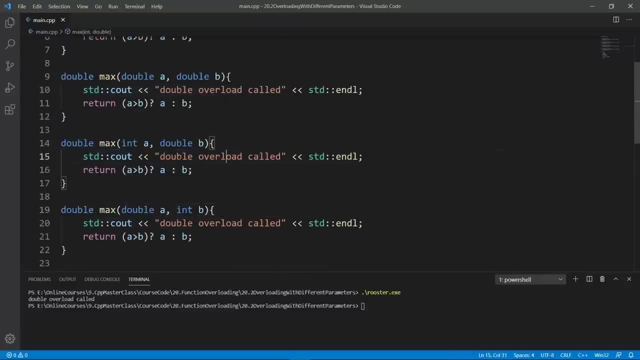 so that you can use it to your advantage. if it makes sense for whatever application you are designing here, so let's go down and put in meaningful output. i think we can come in here and say the parameters that we are passing in here, so we can say ant double overload called. 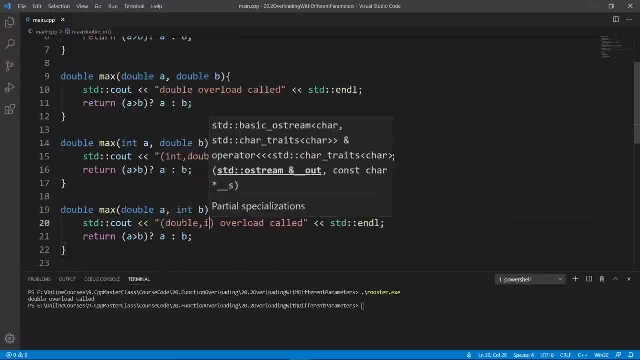 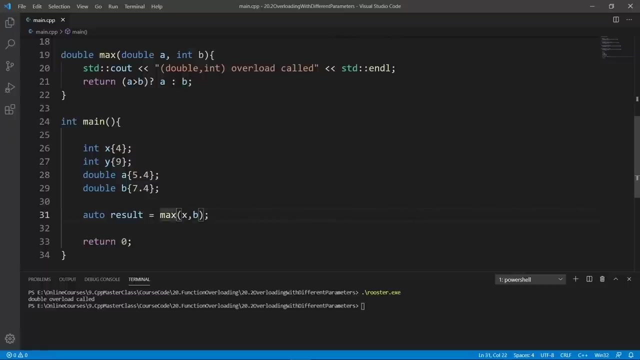 and if we go down here we can take this out and say double and overload called. and to get any of these guys to be called we have to pass the parameters or the arguments in this order. so if we pass in an int which is x- x is an end- and we pass in a double which is a, b, here this is going to call. 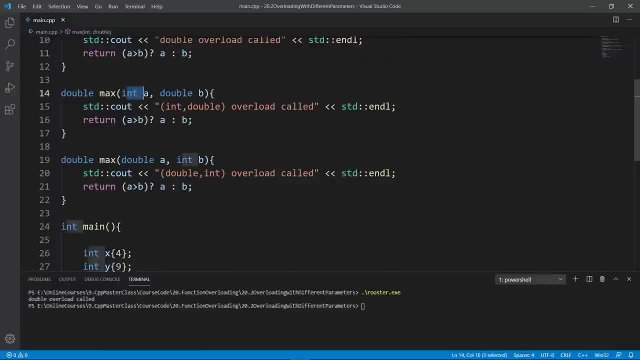 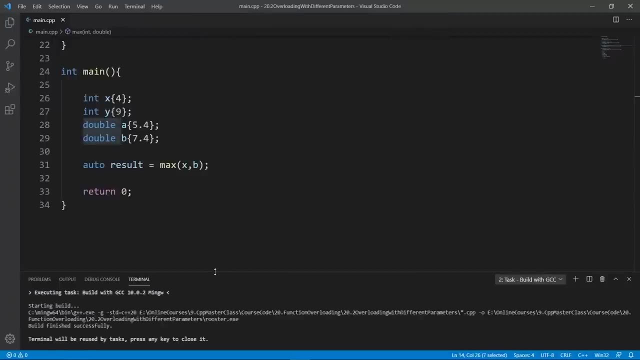 our overload, which takes the first argument to be an integer and the second argument to be double. let's prove that we're going to build with the gcc. the board is good so we can clear and we can run rooster and we see, and double called because x is an int and b is a double. if we flip these, 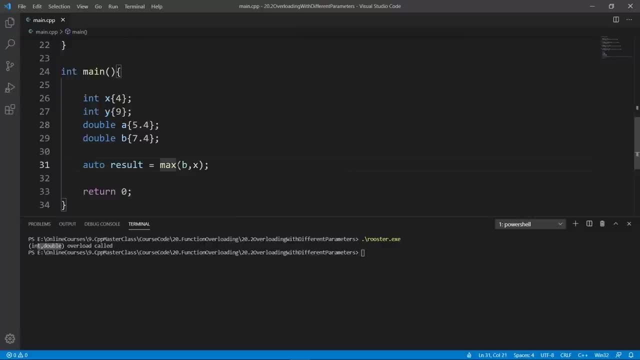 guys. let's say b and x, then we're going to have the overload that takes the first argument of double type and the second argument of intertype to be called, and that's this guy here, and we're going to see this message printed out on the terminal here. let's build with gcc to really 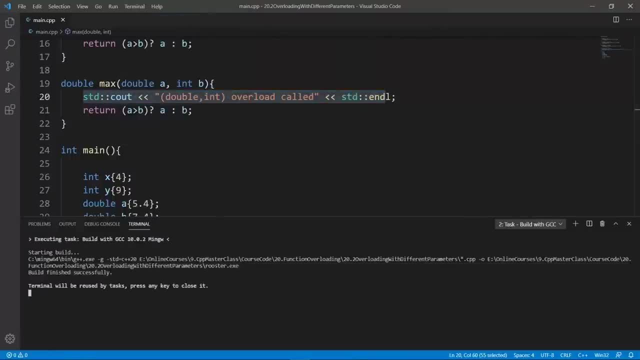 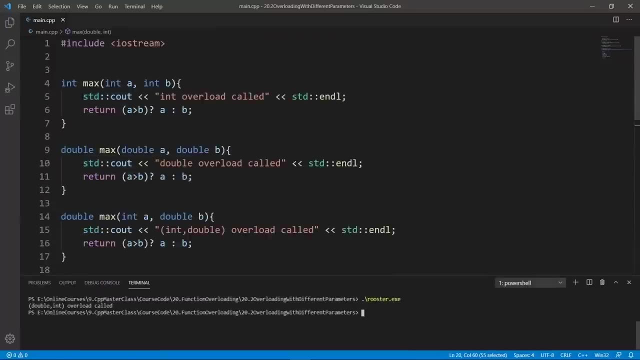 prove this. so we're going to do that. the build is good. we can clear and run rooster and double end overload called. hopefully you can really see that you can set up all kinds of crazy overloads for your functions. the next thing i want you to see is that we can. 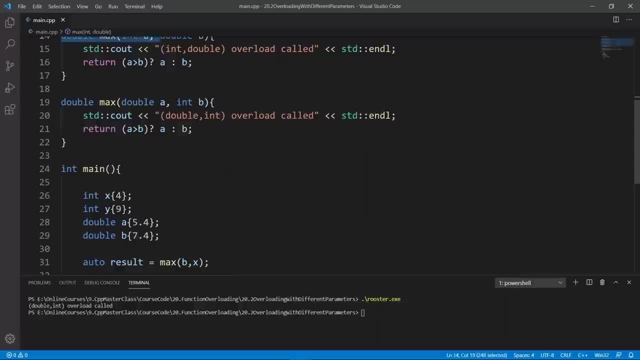 even change the number of the parameters. for example here we can set up another guy here and i call it max. it is going to be exactly like the one on top here for the first two parameters, but let's add a third parameter. maybe make it an end and say c. 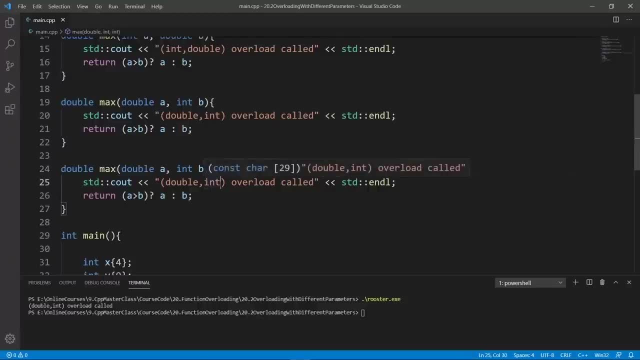 and this is going to be a valid overload for the max function here. so we're going to say double int, and because it takes three parameters, i won't go into the details of how we can compute the maximum between these three guys. what i really am interested in is showing you that you can set up overloads here. 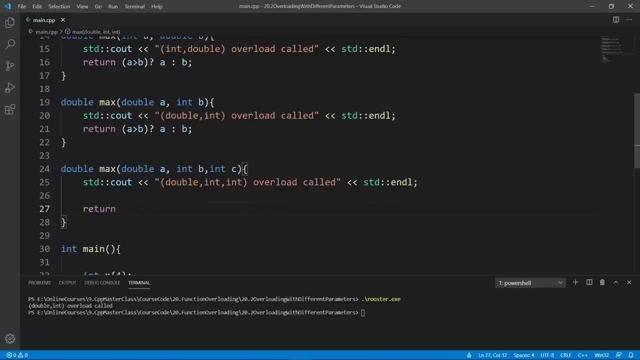 so for this case, we are just going to return. let's just say a. this is going to work, but this is a valid overload for the max function and it is going to compile. so let's draw and do that. we're going to pass on a double, an end and a net, so we're going to pass in b, which. 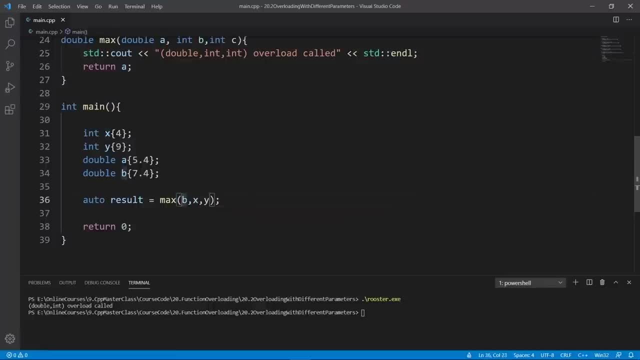 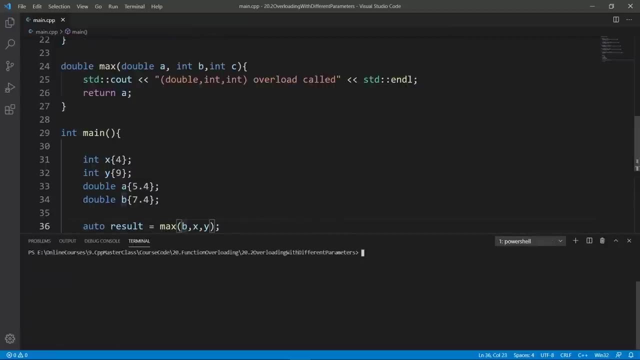 is a double and x and y. let's see what is called here. we can compile with gcc. the world is good, we can clear, and please try to come up with what is going to be printed out here. what is going to be printed? okay, now that you have guessed, we're going to run and we're going to see double int. 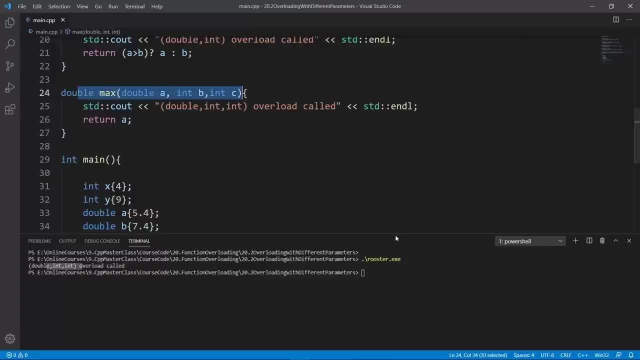 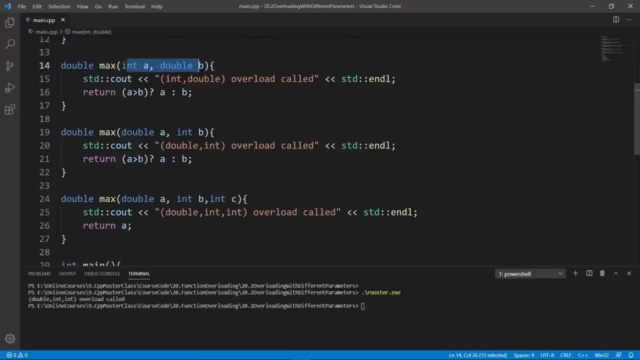 and because this is going to call this overload again, you can overload based on the differences in the parameters that you pass. you can change the order of the parameters, like we are doing here- double and and double- or you can even change the number of the parameters using these techniques. 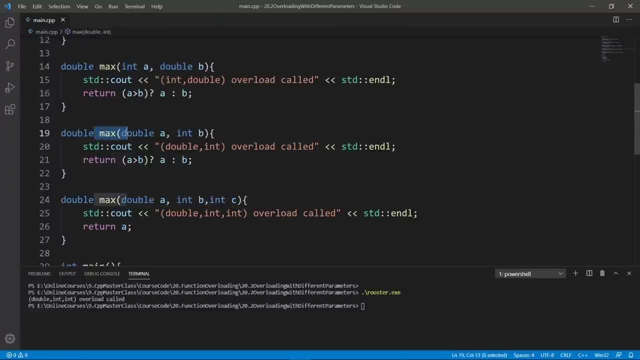 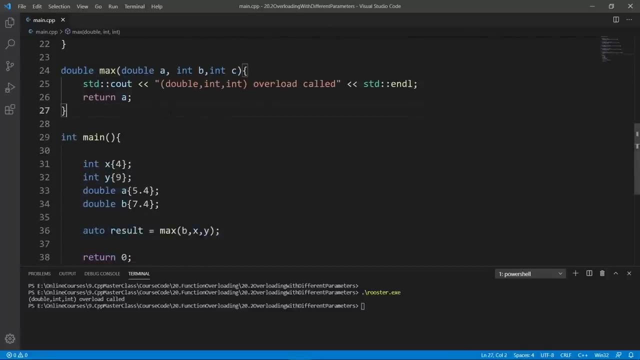 you can make sure that your overloads are different in some way. before i close this lecture, i'm going to show you that you can also use another overload that takes string view parameters. let's go down here and put that in again. the name of the function is max. 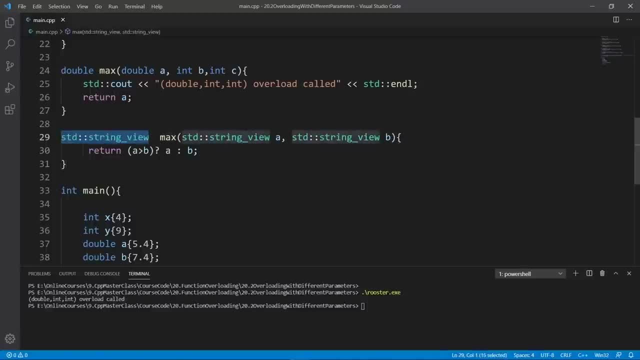 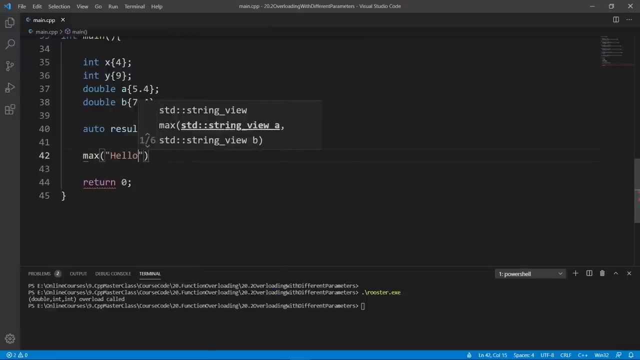 the return type isn't really meaningful in making sure two functions are different. but watch the parameters we pass here. the types are string view and we have a and b here and we are going to compute the maximum. so if we go down here and say max and pass, and hello and world, the 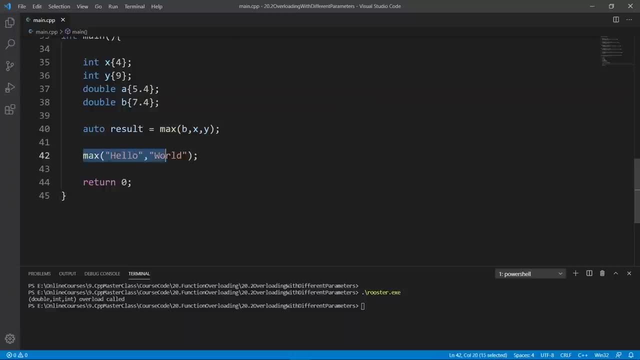 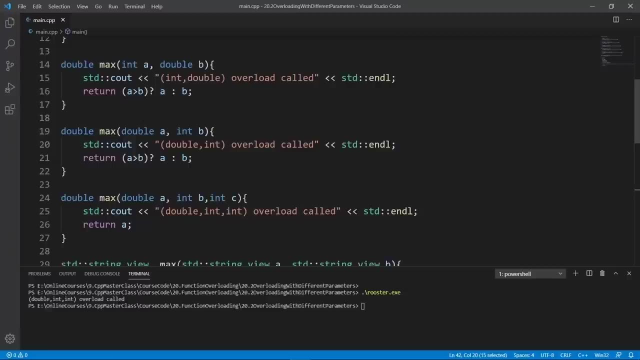 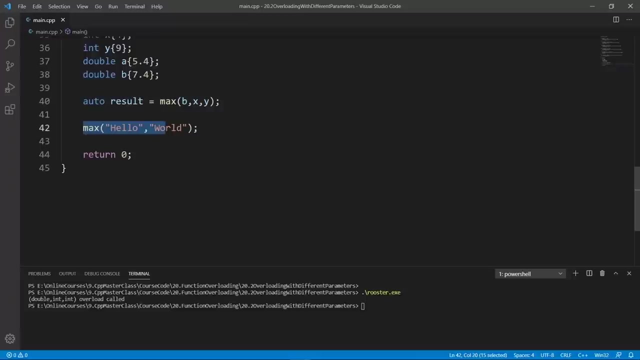 compiler is going to try and look for a function that takes two character array parameters. it's not going to find it because we don't have that guy in here, but it's going to see which function take something i can come up with through implicit conversions and the compiler is going to. 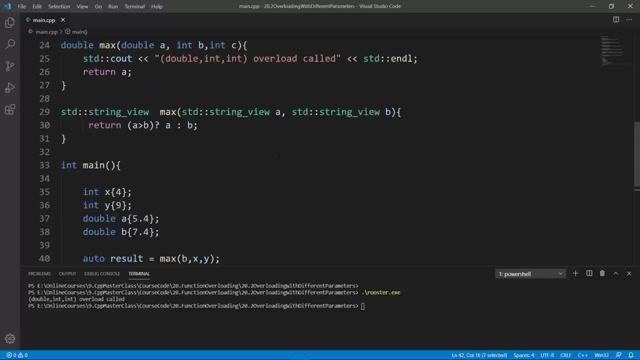 see that it can really convert from a string literal to a string view type and it is going to insert an implicit conversion from string literal to string view and this function here is going to be called. so we're going to put in a an output statement. here we're going to say string view. 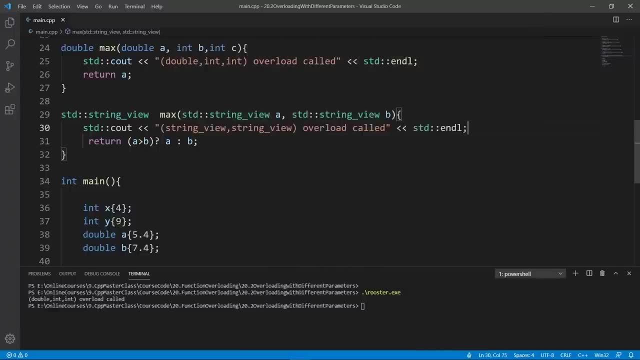 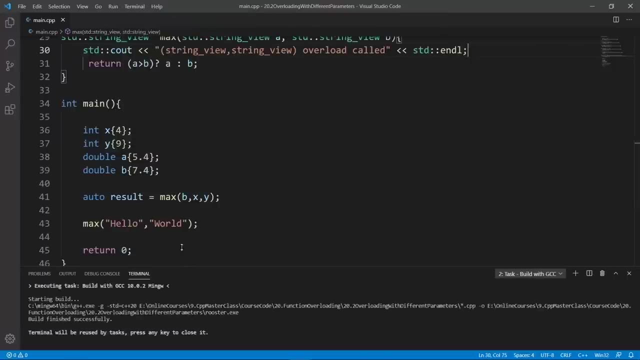 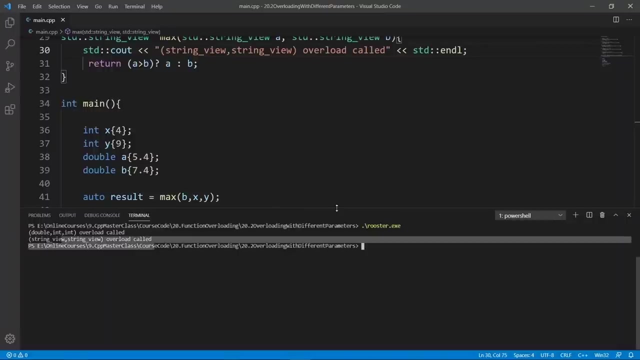 string view: overload cold. and if we try and run this program, let's build with gcc. make sure that the build is good. the build is good so we can clear and run rooster. this is going to show string view. string view: overload cold. we are able to call this guy here and again. the message is that we really have a lot. 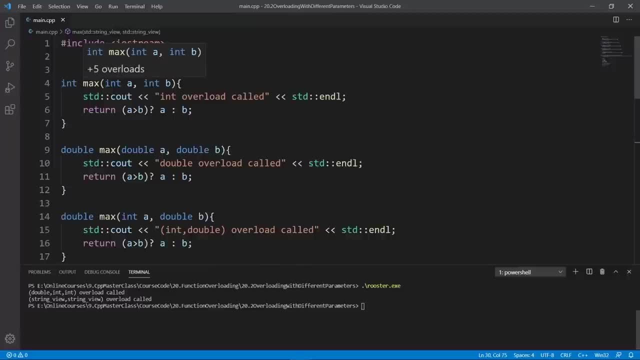 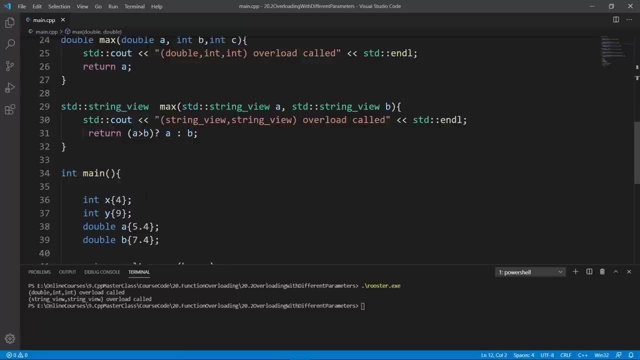 of flexibility in how we can set up overloads for a function in c plus plus, and please use this facility to your advantage. if this is your advantage, you can use this facility to your advantage. if this makes things better for whatever application you are designing, i would like to welcome you in this. 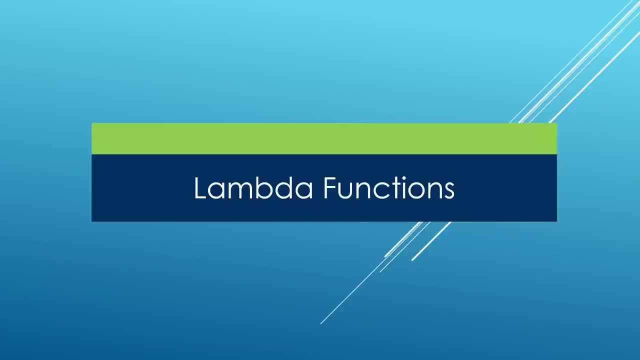 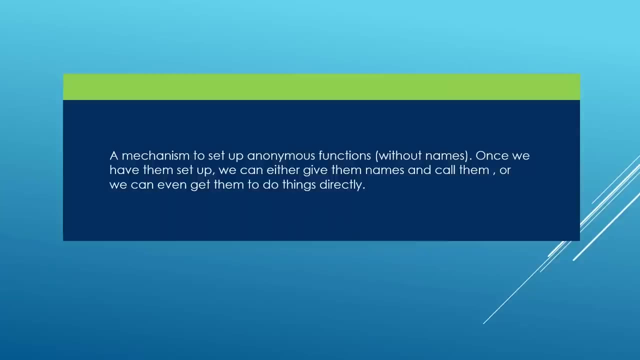 new chapter where we're going to be learning about lambda functions. lambda functions are a mechanism we have in c plus plus to set up anonymous functions. once we have anonymous functions set up, we can do all kinds of crazy things with them. for example, we can give them names and call. 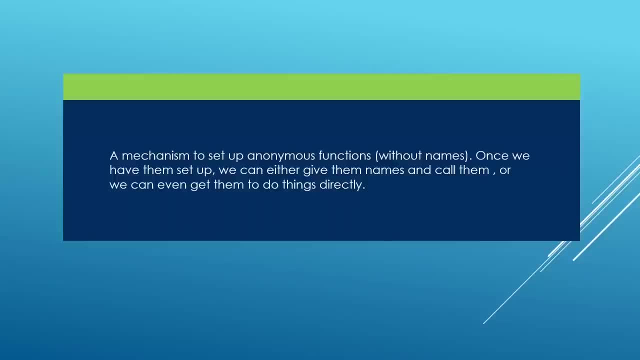 them multiple times, or we can even call them directly without even giving them a name. i realize this can be really cryptic, so we're going to head over to the next lecture and see how we can declare and use our lambda functions. go ahead and finish up here and 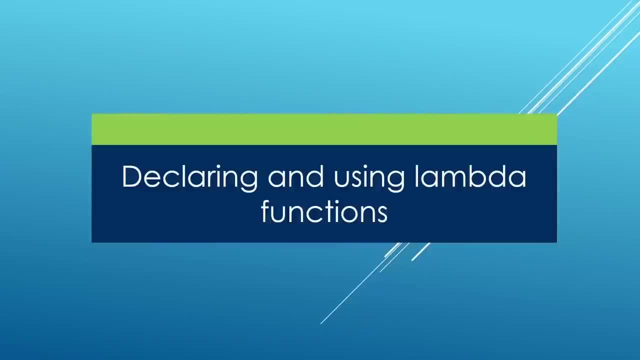 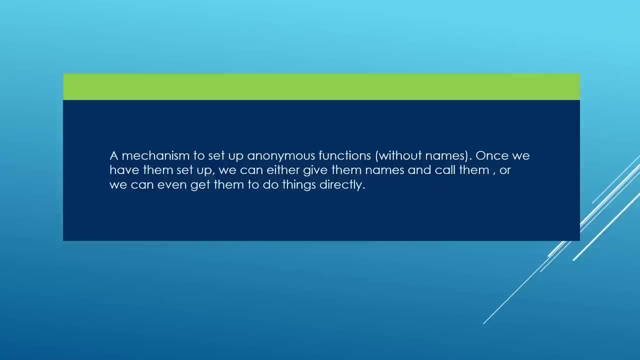 meet me there. in this lecture we're going to see how we can declare and use our lambda functions. and again, lambda functions are a mechanism we have in c plus plus to set up anonymous functions, and an anonymous function is a function without a name. we're going to see how we can set up. 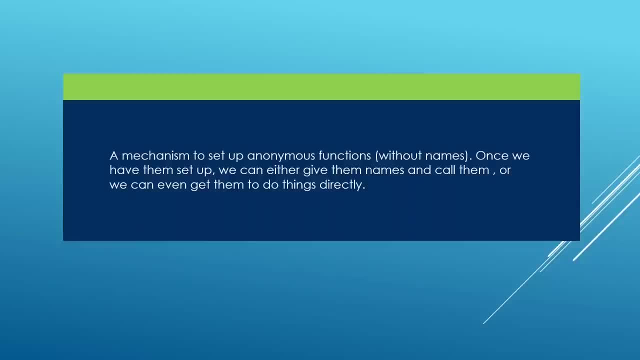 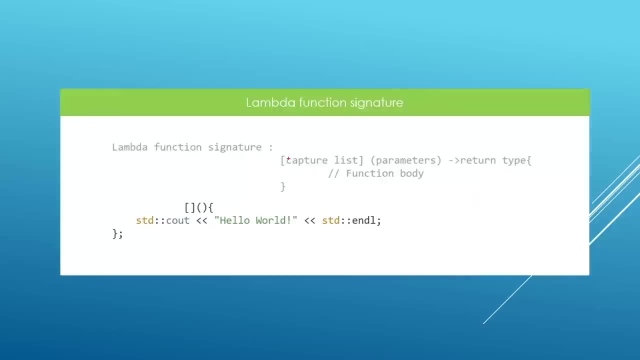 anonymous function. optionally. give it a name and call it, or we can even call it directly without giving that a name. let's see how we can do that. before we talk about anything about lambda functions, we're going to first see the lambda function signature and there is a special syntax. 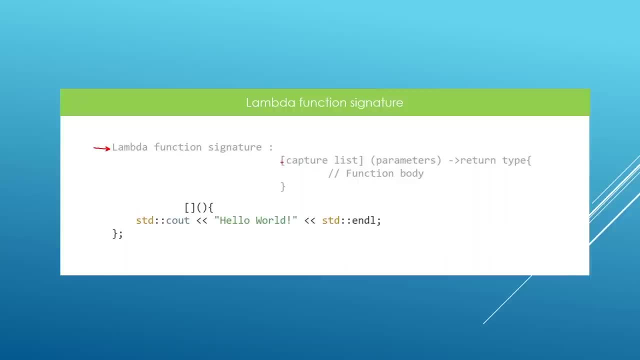 you have to follow if you want to set up a lambda function in c plus plus, the first thing you have to put in place is angle brackets like this, and that's going to be your capture list. we are not going to talk any more about this. we're going to have a chance to talk about this in detail. 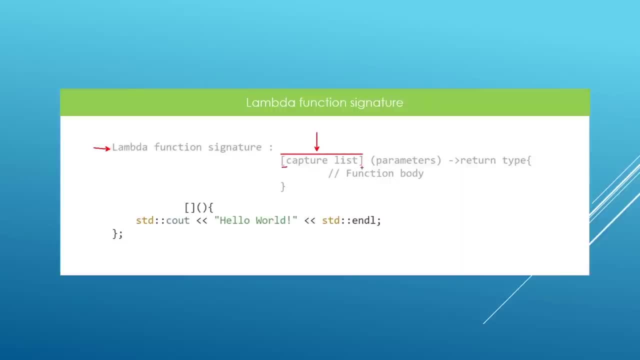 after your capture list, which is going to leave in this pair of angle brackets, you're going to have the parameters to your lambda functions and this is where you can pass arguments if you want to call your lambda function. after that, you're going to have a return type for your lambda. 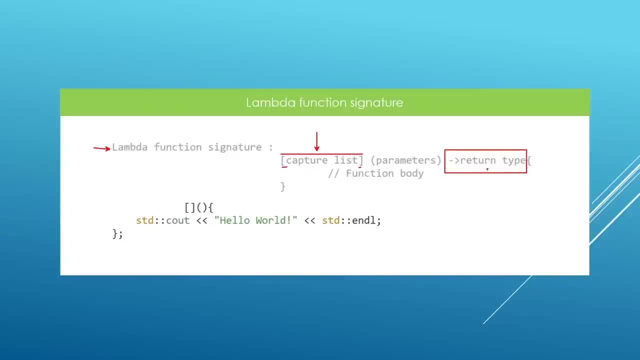 function, but you don't have to put this in explicitly. you can leave this out and the compiler is going to deduce your return type by that itself. after all these things, you have to put in a pair of curly braces and inside these curly braces we're going to have our function body and we can do whatever we want our lambda function to. 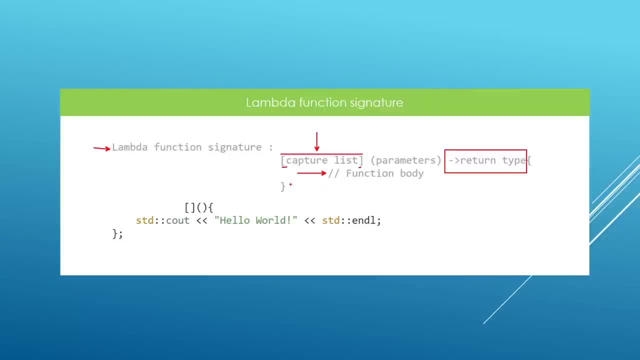 do in this function body here. after this, you will have to remember to put your semicolon to make whatever statements contain this lambda function to be valid, and this is the syntax you have to follow here. we have a simple example. so we have our lambda function, we want to say hello to the 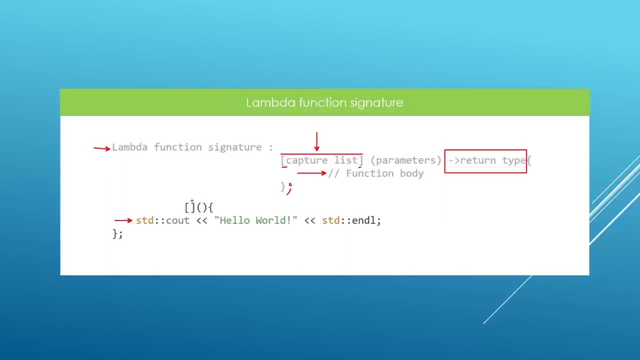 console. this is what we have in the body of the lambda function, but notice that we have our capture list, which is going to be delimited by these angle brackets. we have our parameter list, which is going to be empty in this moment because this lambda function doesn't take any parameter, and we have 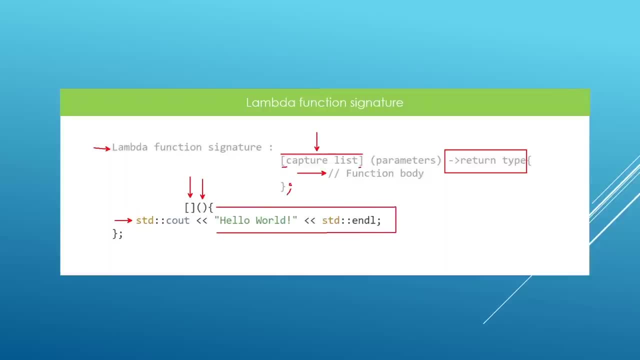 our body, which is going to live within these two curly braces, you. after that, we have our semicolon to make this a valid C++ statement. If we try and put this thing in our C++ source code, this is going to be a valid lambda function, but it isn't really useful by now. 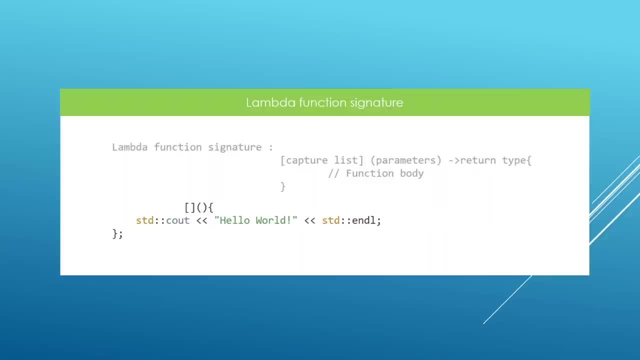 because we can't call it. One way we have to call it is to give it a name, and we can give it a name by assigning our lambda function to a variable, like we see here. Once we have our lambda function declared like this, this entire thing is going to be our lambda function type. We can take this: 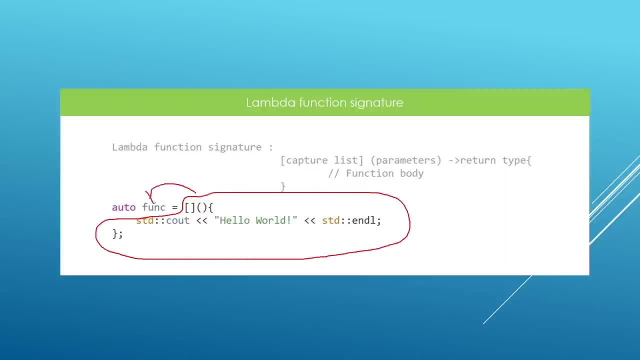 and assign that to a variable which is going to deduce the type using auto type deduction here. This is what we are doing. Once this thing has a name, then we can call it with the syntax we have here, and if we run this code now, it is going to print hello world to the console. I realize this. 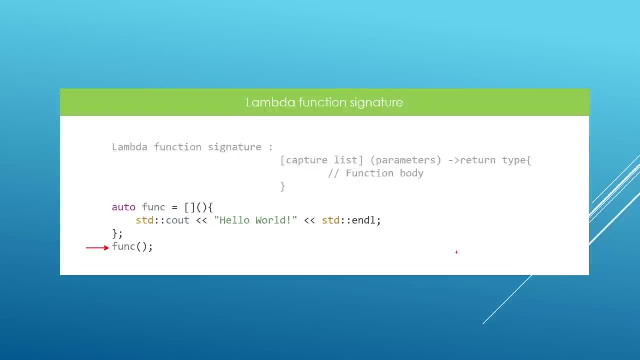 can be really cryptic, but if you try to remember this, you're going to find that lambda functions are really cool, and later in the course we will see that they really make a lot of things easier in C++. So try to remember the syntax here and everything is going to flow from here Again. the syntax is to have the capture list, which is: 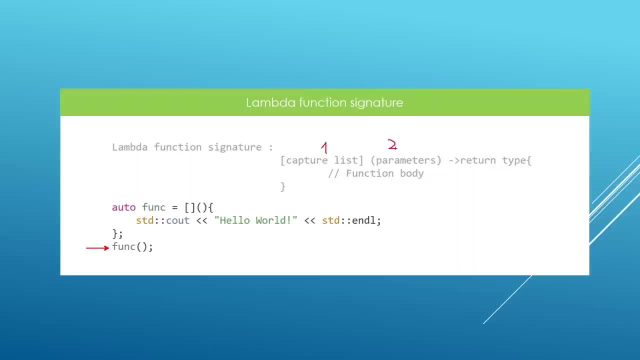 going to be the first thing. The second thing is going to be the parameters. The third thing is going to be the return type, which is optional. You can leave this out and the compiler is going to deduce this and after this, you're going to see that it's going to be the return type. So if you 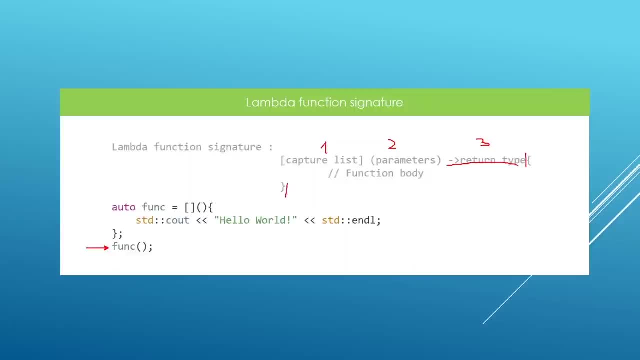 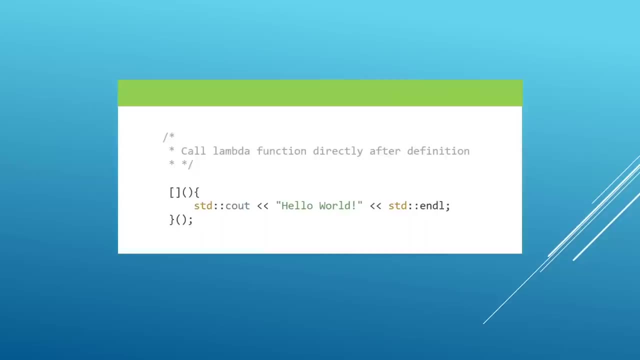 have your pair of curly braces and the body of our lambda function is going to leave within these curly braces. This is the syntax you need to remember. Okay, we have seen that we can give a name to our lambda function and call it, but it is also possible to call our lambda function directly. 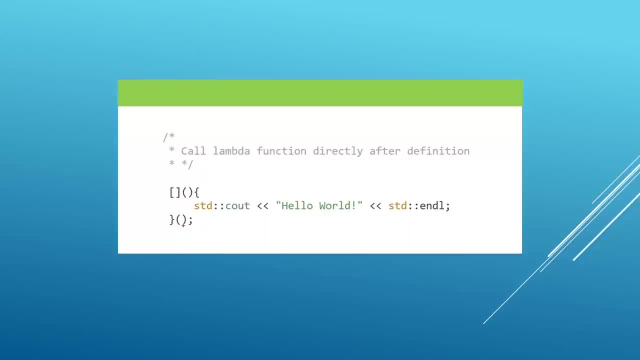 without giving it a name, and we do that by appending a pair of curly braces to the lambda function definition here. So we have a lambda function, we have our curly braces and we have a parameter list. we have our body here and after the closing curly brace we're going to add a pair. 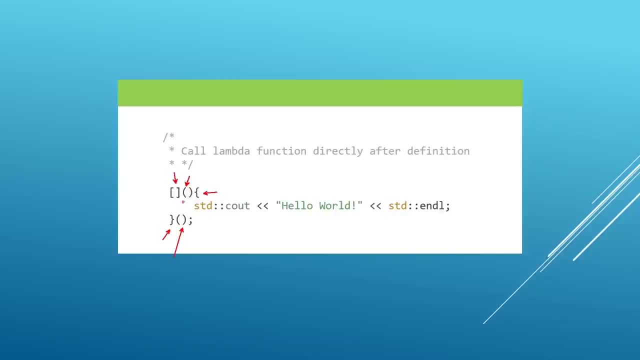 of parentheses to call this lambda function, and because this lambda function takes no parameter, we're not going to put any argument within our parentheses here and this is going to call our lambda function. Don't worry if you find this confusing. we're going to head over to Visual. 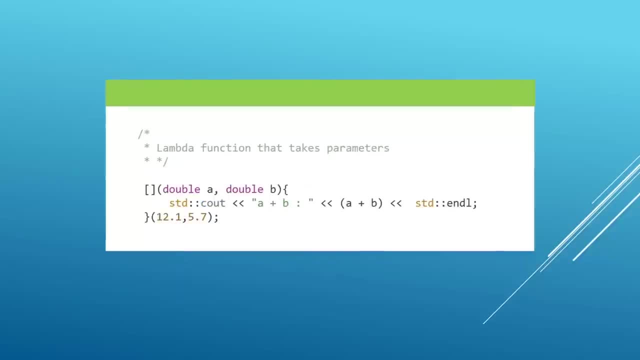 Studio Code in a minute and all of this is going to make sense. Okay, so far we haven't really seen that much of a difference between the parameter list and the parameter function, So we're going to pass parameters to our lambda function. Here is a simple example that takes parameters. This is a 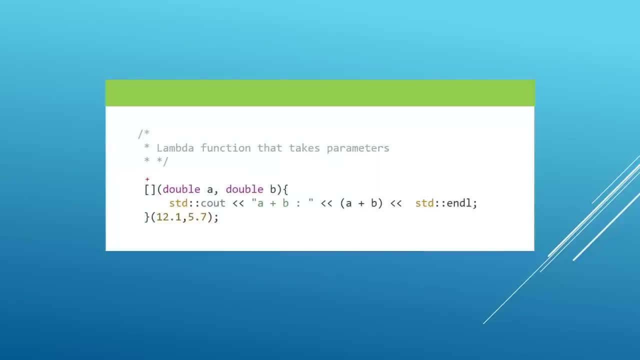 lambda function because it follows the syntax for lambda functions. We have our capture list, we have our parameter list, we have our curly braces and the body is going to live inside these guys and we are calling this lambda function directly with this parameter list. The lambda function is going. 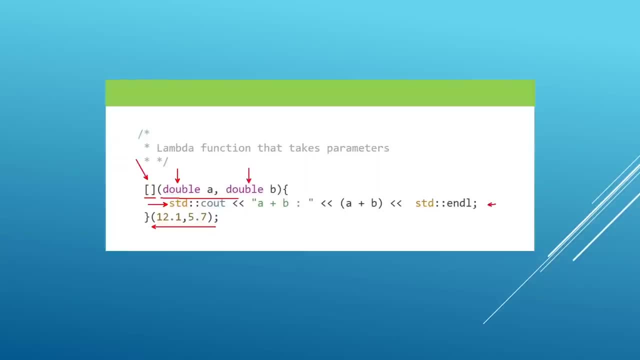 to take two parameters of double type. We're going to print out the sum of these two numbers and we are going to call this lambda function directly. Notice that we are passing in our arguments as double literals. Okay, this is how you can set up a lambda function that takes: 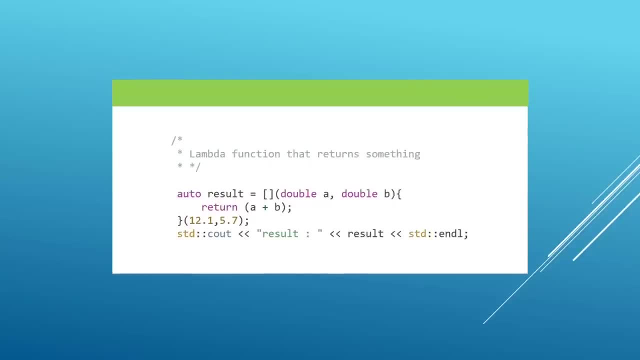 parameters and call it directly. Another thing we can do is make our lambda function return something, and that's really simple. We're going to set up the lambda function like this, so it's going to take two parameters, a and b, and here you see that we are returning a and b, So we're going to 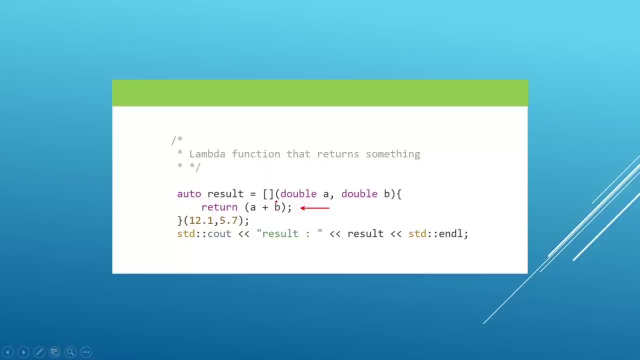 return a plus b, and we can do that. The lambda function is now going to return something, and this entire thing we have here is going to be a lambda expression. The lambda function is going to be called, it is going to return something, and what the lambda function returns is going to be assigned. 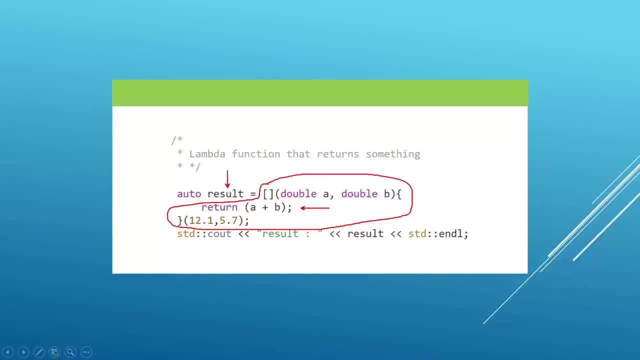 to this result variable here and if we print it, we're going to get the sum of whatever we pass in here printed out on the console and we're going to see it printed out on the terminal. It is also possible to put a number in here and we're going to get a number in here and we're going to get a. 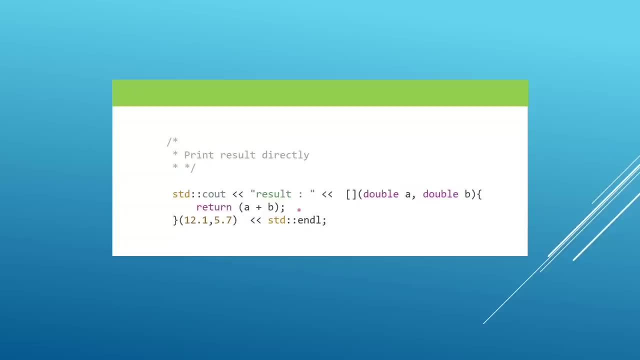 number in here and we're going to get a number in here. So if you click on this one, put your lambda function directly in an output statement. I realize this can be really confusing, but please look at this entire lambda function thing here as a single value, because this is a lambda function that is. 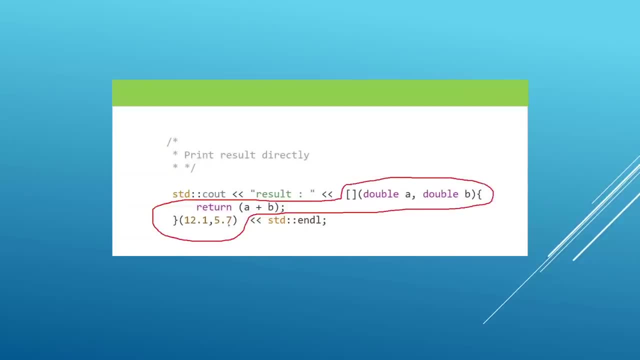 going to return something, and what is returned by this lambda function is going to be printed as our result. here Again- I realize this may be confusing to many of you guys- We are going to head over to Visual Studio Code and let's see what we can do here. We are going to go to the virtual 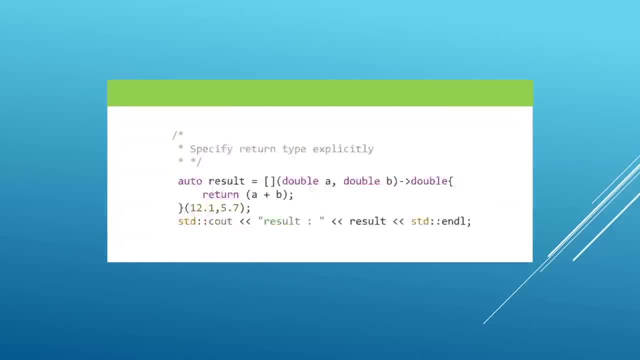 code in a minute and we're going to see this and you're going to really understand. okay, the last thing we're going to look at is that we can specify a return type to our lambda function, and the syntax to do this is to do a dash, a greater than symbol, and put your type after that. 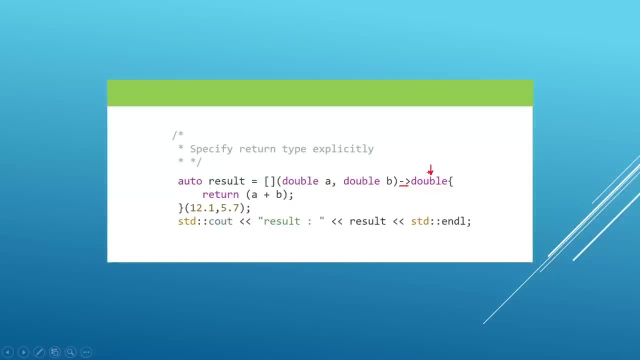 and when you do that now, this lambda function is going to be forced to return double type, even if you pass it to parameters that are not of double type. we are going to add them up and the return type is going to be implicitly converted to double, and that's what we're going to return and we can. 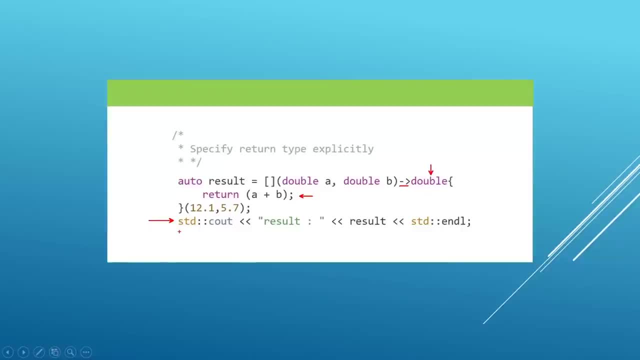 print it out on the console, and we're going to see an example of this in a minute- when we hit visual studio code. in fact, this is really all i had to share with you in the slides. i realize many of these things may be confusing. we are going to head over to visual studio code and play with. 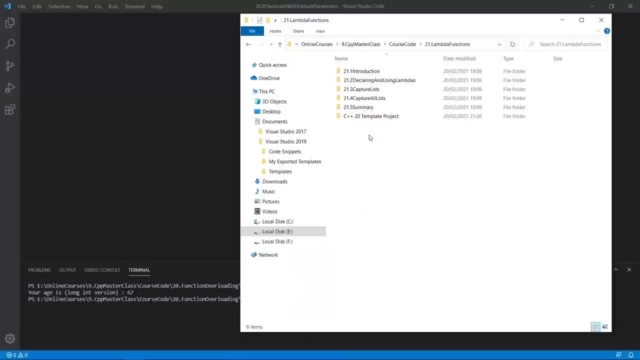 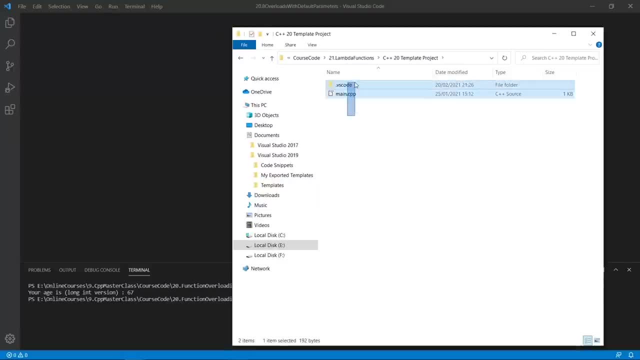 these things step by step. you am sure you're going to understand. here we are in our working directory. the current project is declaring and using lambda functions. we're going to grab our template files and put them in place. let's do that- and we're going to grab our folder here and drag and drop it in visual studio code. 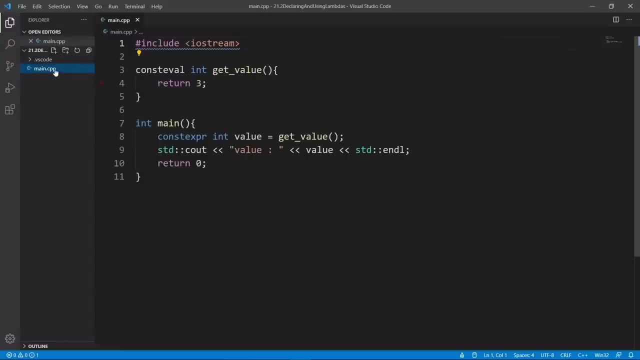 and this is going to open it. it is opened here. we have our main cpp file opened, we can close the left pane here because we don't want it anymore, and we can clean up our function here, and the first thing we're going to do is to put in the syntax for a lambda function here and use it as a reference as 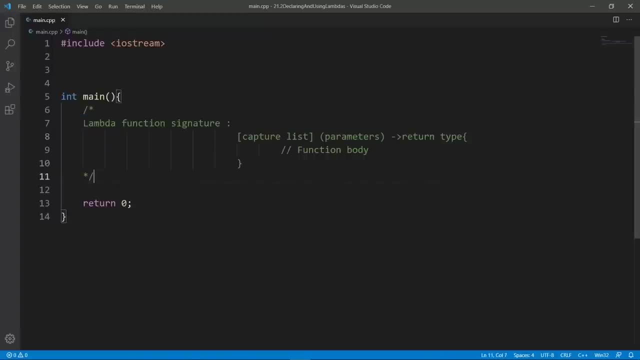 we learn about this. i think this is going to make things a little easier. so the first thing we want to do is to declare a lambda function, and the first thing we need to put in is a capture list. a capture list is going to be englobed in this angle bracket, so this is our empty capture list. 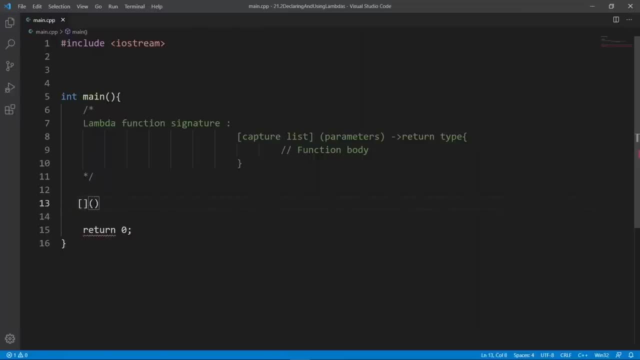 and after this, we're going to put in a parameter list which is going to leave inside these parentheses here. After that, we're going to put in an optional return type. For now, we're going to ignore this, And after that we're going to put in our pair of curly braces. 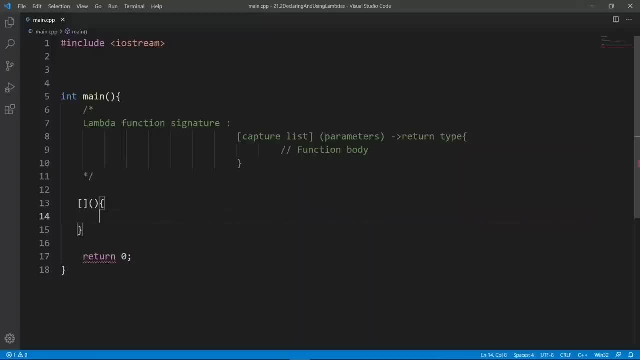 And inside this pair of curly braces is where the body of our lambda function is going to leave. So inside here we can do whatever we want. in the body of this lambda function, For example, we can say hello world, which is the logical thing to do at this point. 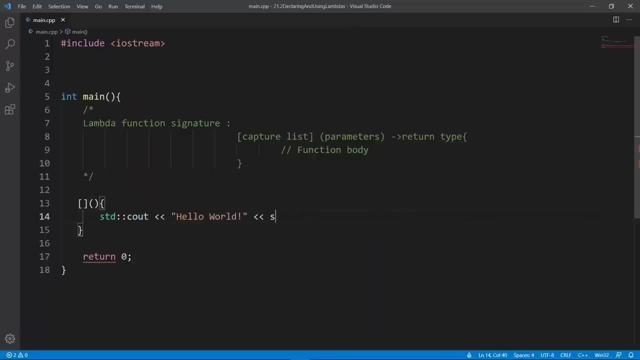 So we're going to say hello world here And we're going to put in our new line character with ENDL. Okay, now we have a lambda function declared, But we have to put in a closing semicolon because this is a C++ statement. 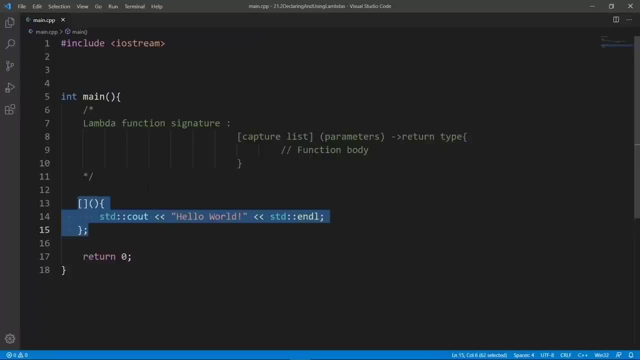 Okay, now we have our lambda function declared And this is valid C++ code. If we're trying to compile this program, you're going to see that it is going to compile. fine, Okay, world finished successfully. And if we're trying to run it, it is not going to do a thing. 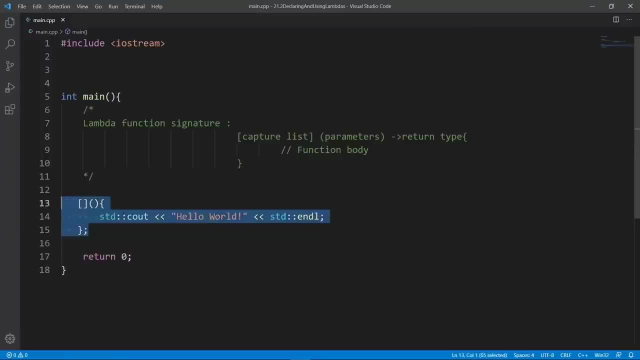 Because we are. We are declaring the lambda function here, but we're not calling it to get it to do things. So let's bring up a terminal and show you that if we run this program it is not going to do anything. So let's do clear and run rooster. 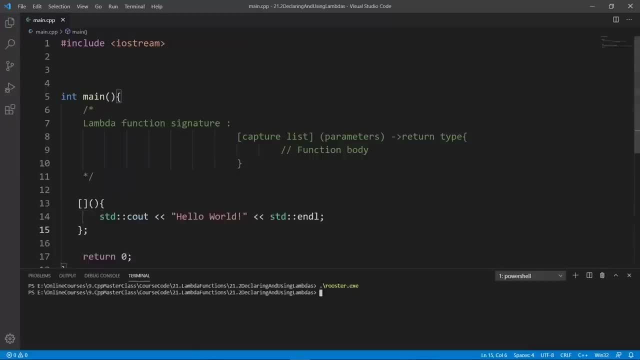 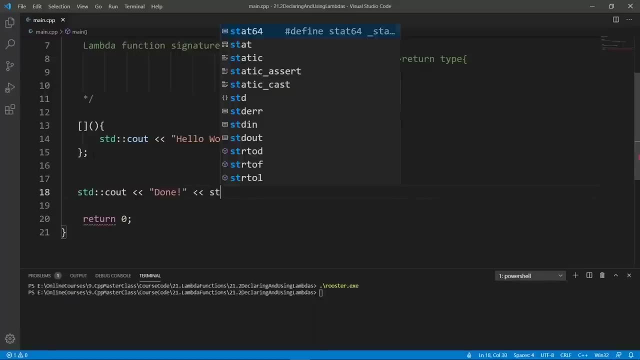 You're going to see that it's not going to print anything. And we can even go down here and put in a closing stdcout statement saying done, To mean that we are hitting the end of the function here without doing anything. So if we world again, 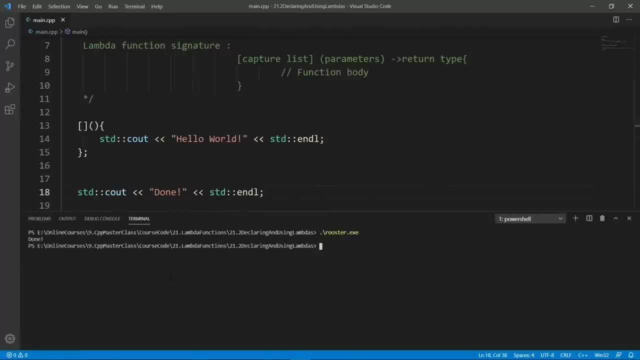 The world is going to begin. Okay, good, We can clear and we're going to run rooster. You see, we are printing done. We are hitting the end of the function here And we're not seeing hello world. So this function here, or this lambda function here, to be exact, is not being called. 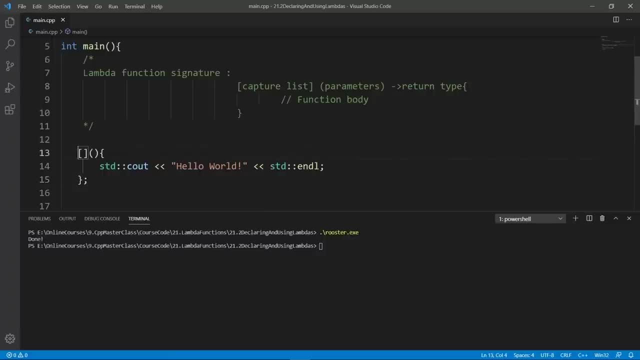 One way we have to call it is to give it a name, And we have seen that to give it a name we have to assign the entire lambda function thing we have here to a variable, And we're going to use auto type deduction here. 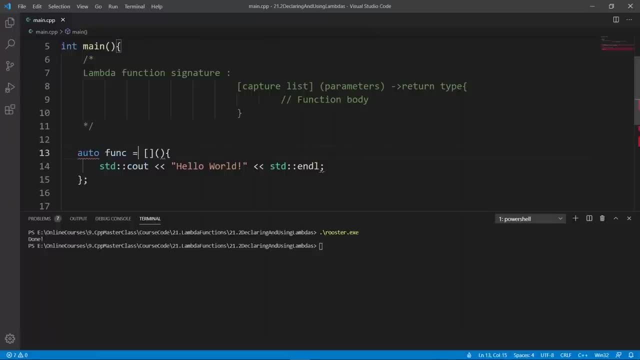 So we're going to say auto function And we're going to assign our lambda function here to this variable And this is going to be basically a handle we have in our program here to the lambda function And we can use this handle to do things with the lambda function. 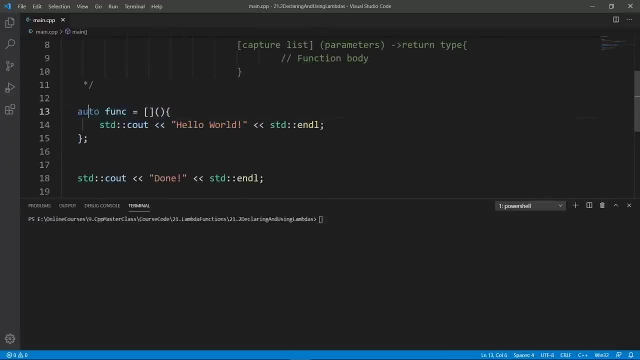 But by now I want you to see that even if we run the program now, it is not going to do anything Because we're still not calling the lambda function here. Let's show you that we're going to world again And the world is going to be good. 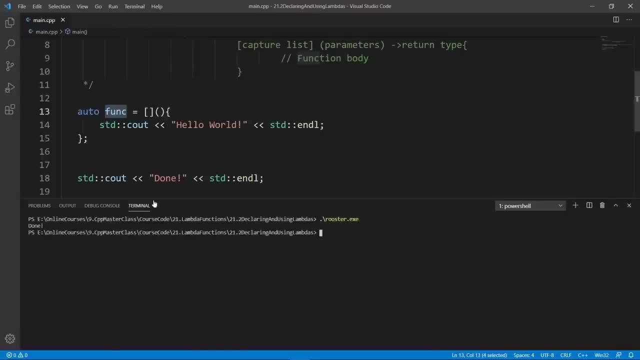 No problem, We can clear and run Rooster. Still no hello world, Because we're not calling our lambda function. To call our lambda function, we have to use our handle here, which is this variable, and use regular function called syntax. 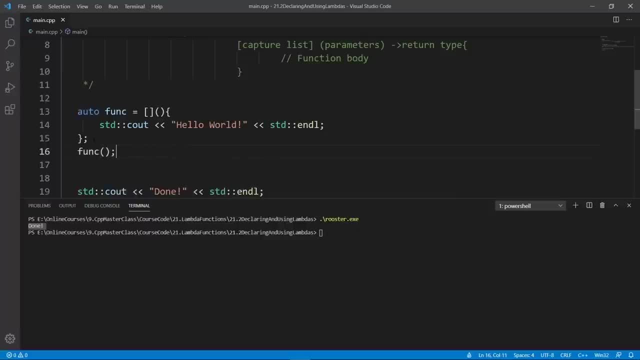 So we can go down here and say func, And we can put in our parenthesis: We're not putting in any parameter, because this lambda here doesn't take any parameters. And now if we run this program, it is going to say hello world. 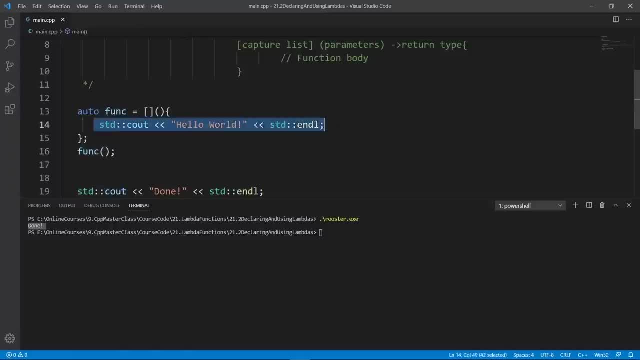 world, because this line here is going to call this lambda function. let's bolt and see that we're going to use gcc to world. so now, if we clear and run rooster, we're going to see hello world. we can call this function multiple times because we have a handle to it. the handle is going to be: 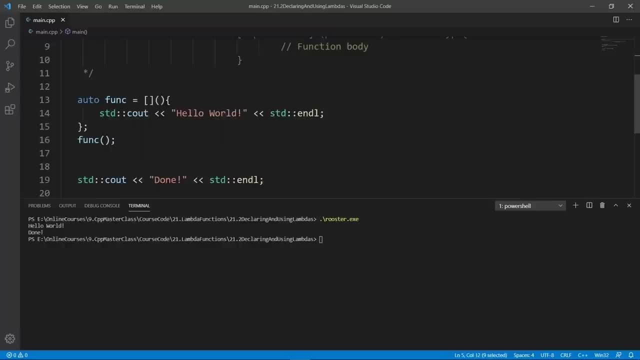 valid throughout the scope of the main function here. so we're going to go down and call it again and if we build, we're going to build with gcc. the build is good, you can clear and run rooster. we're going to say hello world twice because we are calling our lambda function twice. this is one. 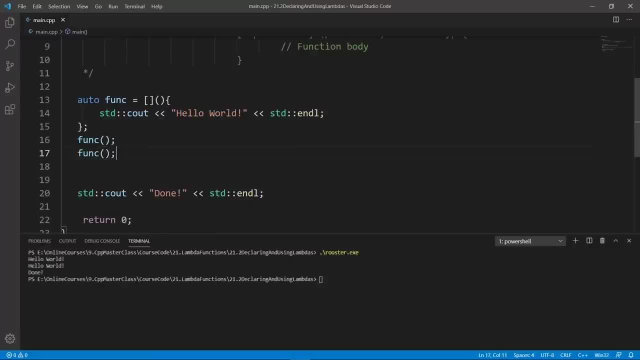 way we have to call our lambda function here. so we're going to comment this out, because we're going to see a few other things and on top here, what we were doing is declaring a lambda function and call it through an a. now we're going to go down, set up a lambda function. 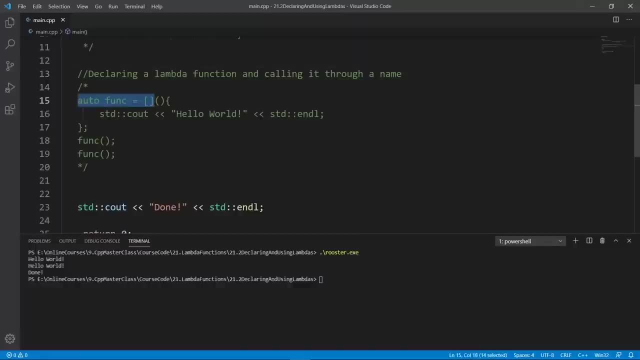 and call it directly, without giving it a name, because that's also a possibility in c plus plus for that we're going to grab our lambda function here and we're going to copy it and we're going to say: declare a lambda function and call it direct. and the syntax to do that is really simple: you set up. 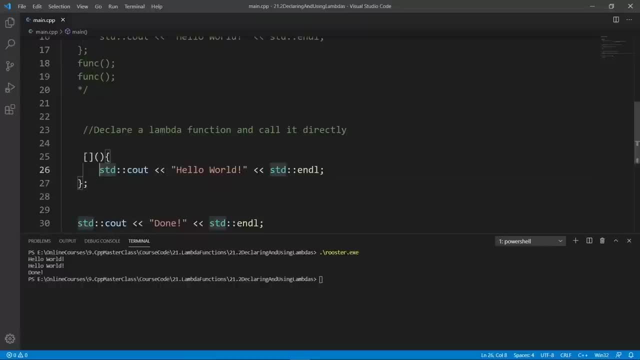 your lambda function, like we have seen before. you see, this is our lambda function statement here, but you're going to go to the closing curly brace and add a pair of parentheses. this is going to declare a lambda function and call it directly, without giving it a name, because that's also a. 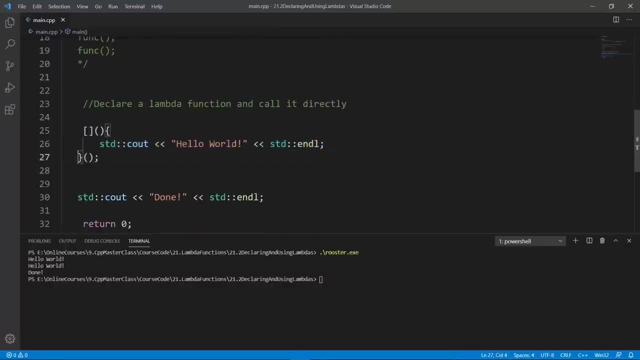 called it directly. notice that we don't have a handle to this lambda function. so if you do things like this, you will have only one chance to call the lambda function. so we're going to say hello world once, because we are declaring the lambda function and calling it directly here and after. 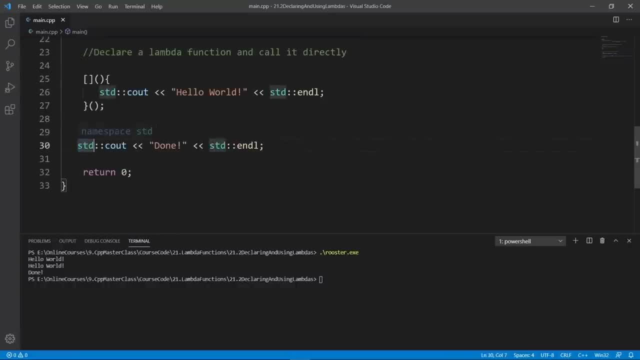 that we're going to say done because we're going to be hitting the end of the main function here. let's build the program and show you that we're going to build with gcc like we always do. we're going to clear and run rooster. this is going to say hello world and we're going to be done here. 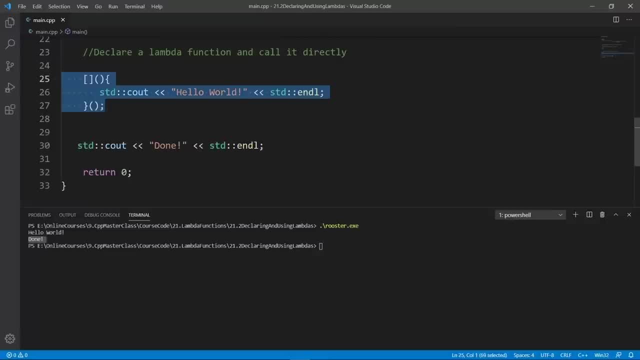 because we are calling this lambda function once again. notice that now we don't have a handle to this lambda function, so we really have one chance to call this, and you will do this if you just want to set up some function that you want to call directly and you don't care about calling it ever. 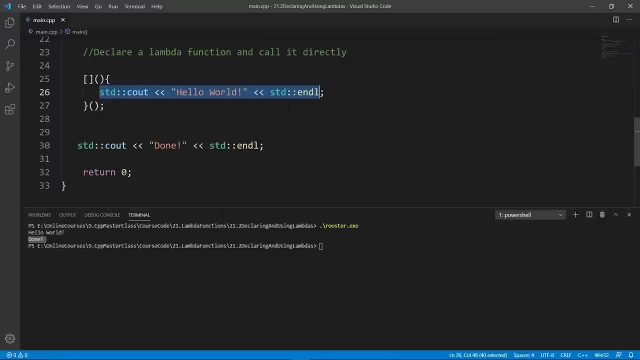 again in your c++ application, and we're going to see that we have many kinds of problems where we want to do these kinds of things. okay, now that you have seen this, the next thing i want to show you is how to set up a lambda function that takes parameters, and we're going to comment out what 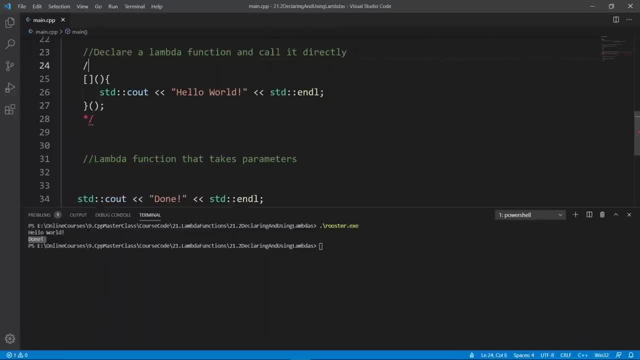 we have on top here, because we don't want noise output on our terminal and we're going to grab this lambda function and adapt it, so let's copy it. we're going to go down here and put it in and we want to pass two parameters. now let's pass in double parameters. we're going to pass in. 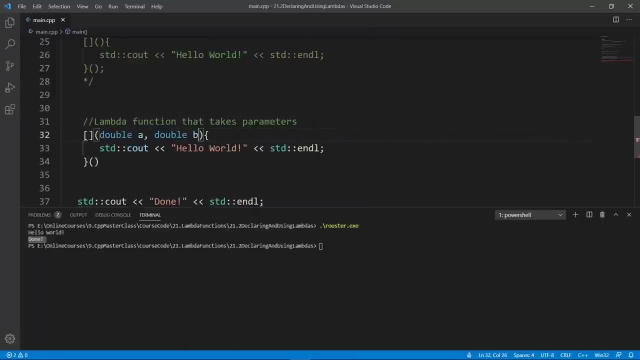 double a and double b. we can do that and inside the lambda function we can print the sum of these two variables. so we're going to say a plus b, for example, and we're going to print out whatever is the result of a plus b. let's do that, and after we do that, you're going to see that we get a compiler. 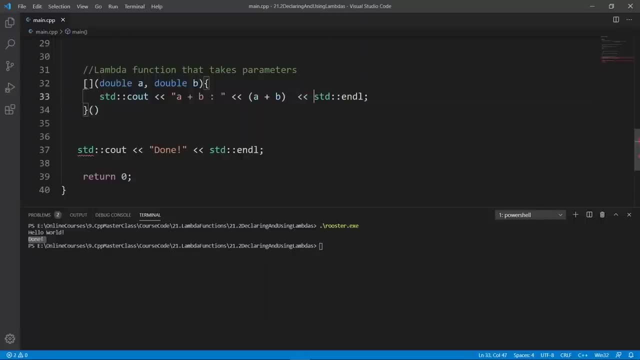 error, because now our lambda function is taking parameters, but we are calling that with an empty list of parameters, so we need to give it something. to sum up, let's give it 10.0, for example, and 5.0 and see what we get, and after this we need to put in. 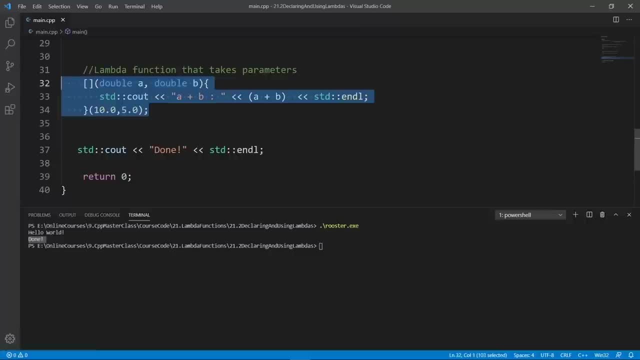 our semicolon, because this is a c++ statement and any c++ statement needs to end with a semicolon. now try to think about what we are doing here. we are setting up a lambda function- okay, it's going to end with a semicolon- and we're going to put in a lambda function and we're going to put in a. 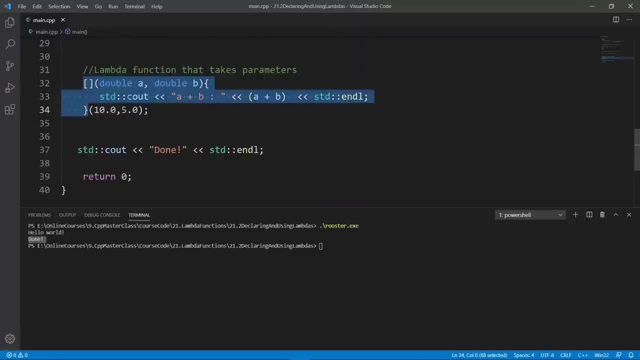 at this closing curly brace, and this lambda function is going to take two parameters of double type and inside the lambda function we are going to print out whatever is the sum of these two parameters that we are taking in here. after that we are calling our lambda function with: 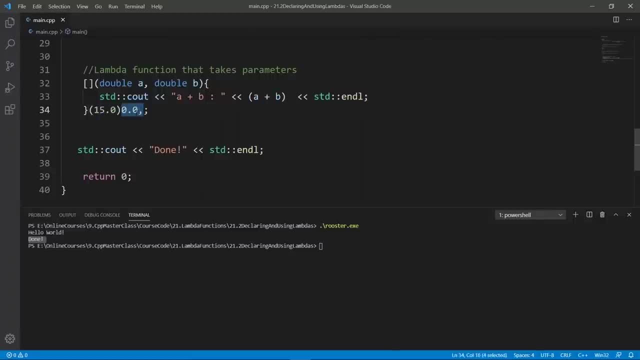 two variables, 10.0 and 5.0, or i should say two double literals. that's what we are calling our function with. and now, if the program runs, the lambda function is going to be called once and we're going to print out whatever is the sum. 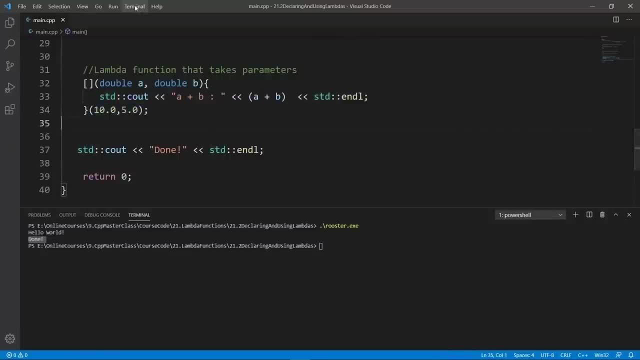 of these two numbers, and that's going to be 15. let's build. so we're going to build with gcc. the build is good, we can clear and run rooster. we're going to see a plus b is 15. we are calling our lambda function here. if we put in a 50 here, for example, we're going to get 60 printed out. 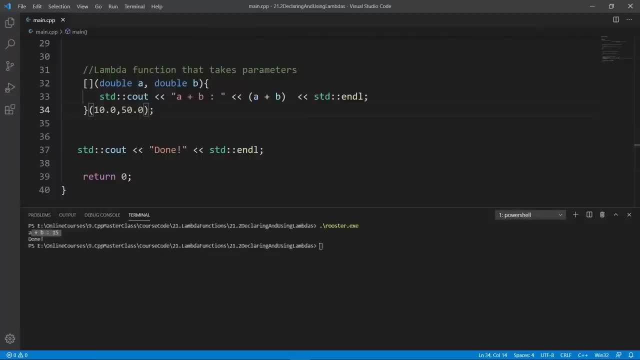 because that's going to be our sum. okay, let's build again and see that printed out. if we run rooster, we're going to see 60 printed out and we're going to see that printed out and we're going to see 60, because that's the sum of 10 and 50 here. another thing we can do is actually not call the. 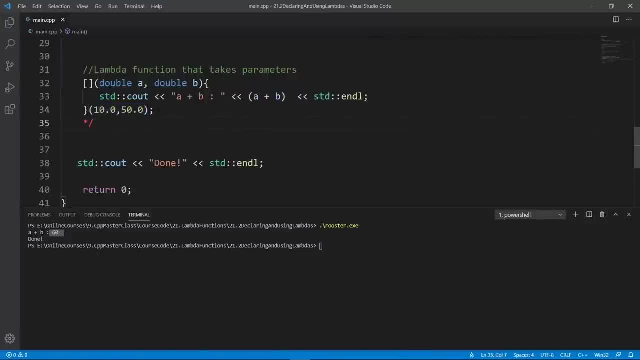 lambda function directly here we can actually comment this out. i don't want to take this out because you might want to use this as a reference. so we're going to comment this out and set up another example that is going to name our lambda function, and then we will have a handle to the 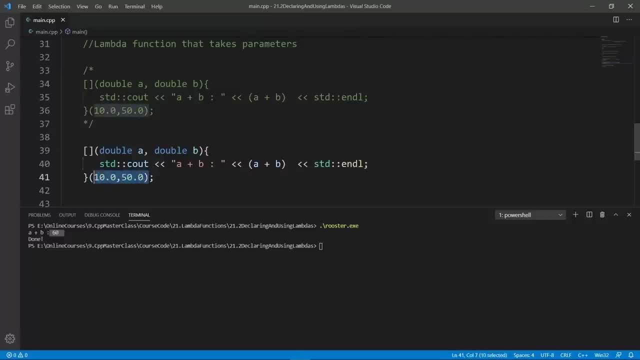 lambda function and we can call it multiple times. so let's take out the call we are doing here and we're going to assign our lambda function to a variable. we're going to say auto func1, we can call this func1, no problem. and now we can call this lambda function multiple times. for example, we can: 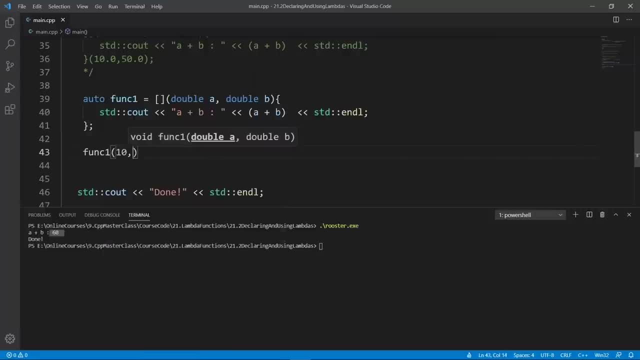 say func1 and pass in 10 and 20. okay, and we can say func1 and pass in 5 and 7. why not? if we run this program, it is going to print the sum of 10 and 20 and it is going to print the sum of 5 and 7. 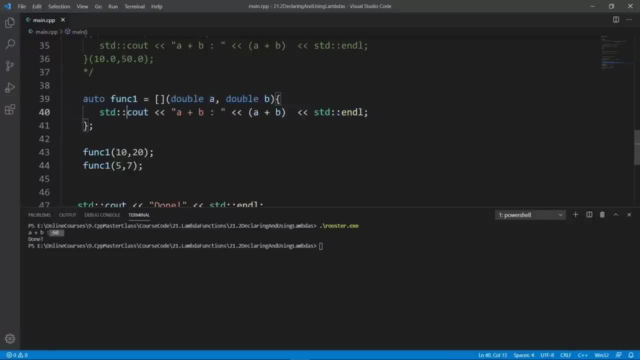 and it is going to be calling this lambda function multiple times. hopefully you can see that if you want a chance to call your lambda function multiple times, you will need to give it a handle, like we are doing here, and then you can use that handle multiple times and call your lambda function. 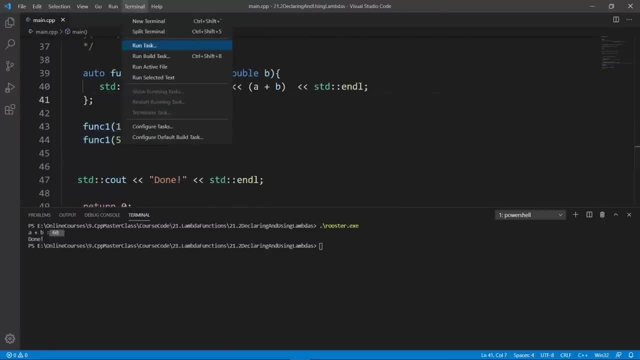 however many times you want. so let's build this program and see what we get on the console. we're going to clear and run rooster now. we're going to see a plus b- it's 30 as a result of this call here. and we're going to see a plus b is 12 as a result of this call here. 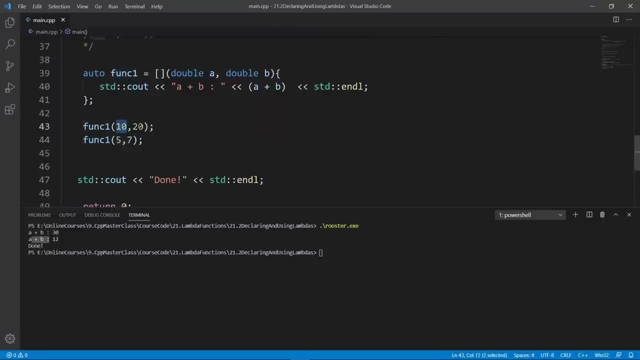 notice that we are passing an integer literals. so the compiler is going to insert an implicit conversion from n to double because our lambda function here is taking double time. you really need to be aware of these implicit conversions and make sure they are working to our advantage. if they are working against you, try to find a way to make you good. 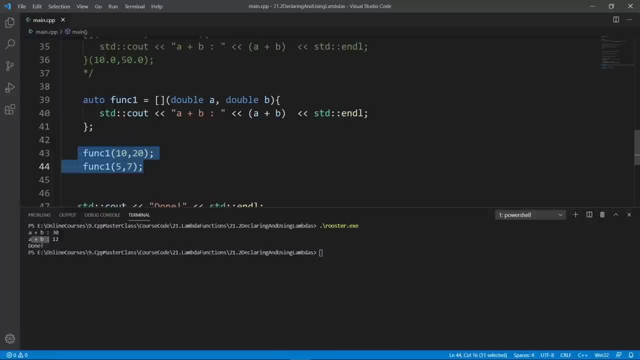 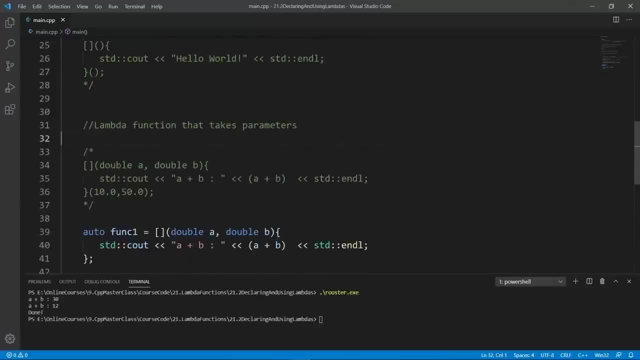 work exactly like you want, because we are learning about all these cool tricks in c++. you're going to be using them at your advantage. okay, hopefully now you know how you can set up a lambda function that takes parameters. we're going to go down and comment this out, because now 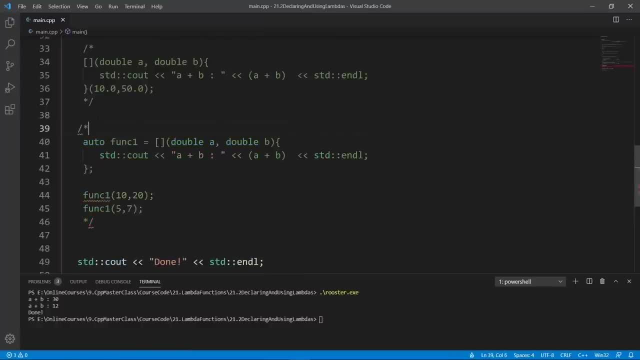 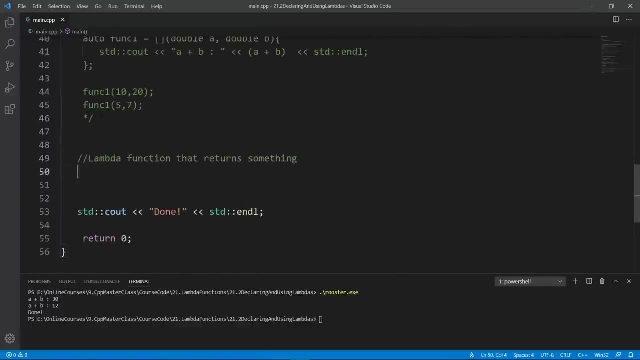 we want to see how we can return something from a lambda function and we're going to be using the same lambda function here. so let's grab it and we're going to say: lambda function that returns something. and we're going to set up our lambda function and we're going to say: lambda function. 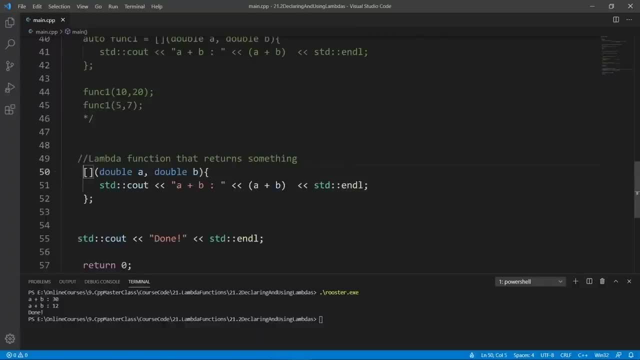 here. let's put that in place correctly and instead of printing out the sum of a and b, we can return that. we can go in our lambda function and say: return a plus b. okay, now that we have this, we can either call it directly by saying, for example, 10 and 20. but now, if we try, 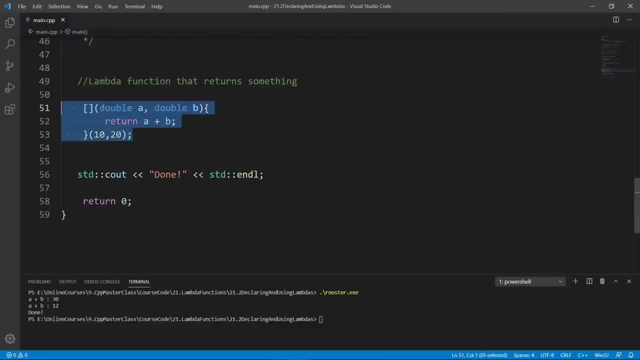 and run this code, it is not going to do anything. try to guess why this lambda function is not printing out the sum of a and b. we can return that. we can go in our lambda function and say: return to the constant directly. it is just returning whatever is the sum of 10 and 20. and if we return, 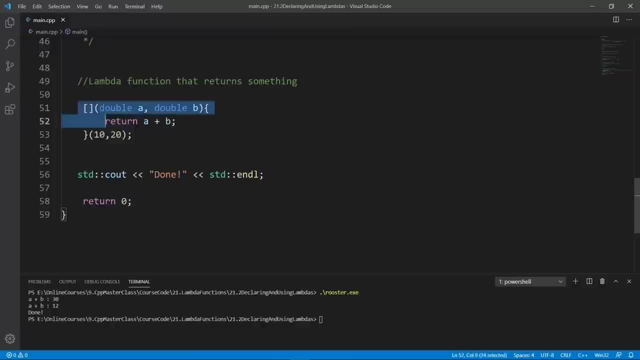 it. we're not doing anything with whatever is returned from this lambda function, so we're not going to print anything and we're just going to print down here. let's vote and make you see this, because you really need to be aware of these little things. so the build is good, we can clear. 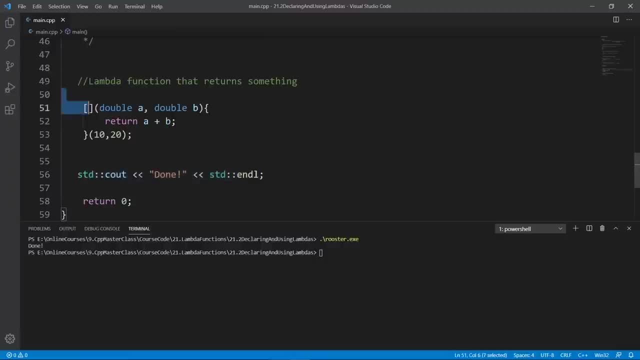 and run rooster. we're going to see done. our lambda function is returning something, but we're not doing anything with the return value. if we want to print the return value, we need to catch it somehow and we can put that in a variable. for example, we can say auto result and assign the return value of our lambda function. 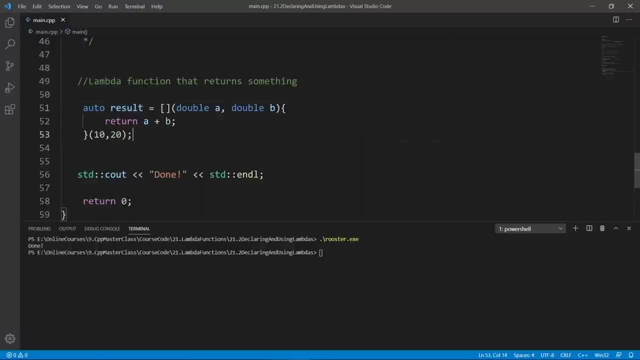 to this variable. now we have a chance to print this, for example, by doing stdc out result, and we're going to print that out and save result. now, if we wrote this program, it is going to print whatever is the sum of 10 and 20. let's do that and show you that this is a result and we're going to 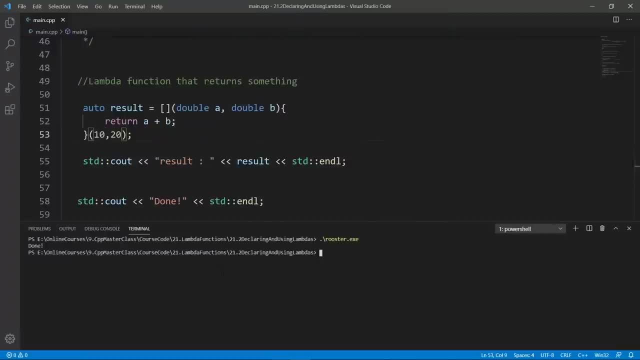 actually the case. so build is good so we can clear and run rooster. result is 30. if we pass in 10 and 50, for example, we're going to get the same thing. let's pass in 60 here. so we're going to build with. 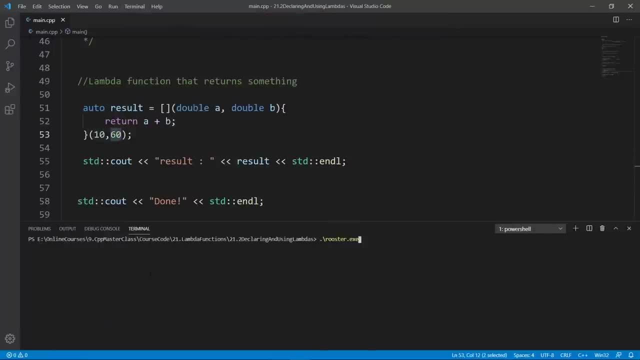 gcc. the build is good. we can clear pretty quick and run rooster. now the sum is 70 and this is how you can return stuff from your lambda function and once you return stuff you have to be sure you catch your rooster and you can print it. so we're going to print this and we're going to 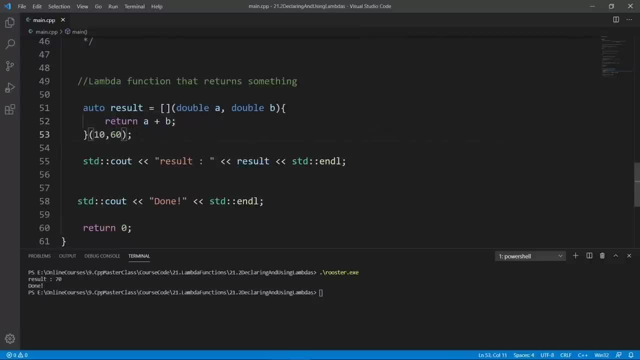 print the result and print them out. another thing you can do is print out the result directly after you call your lambda function. so, for example, we can grab this entire lambda function thing here and put that in an stdc out statement. so we're going to put in a second one here and say result. 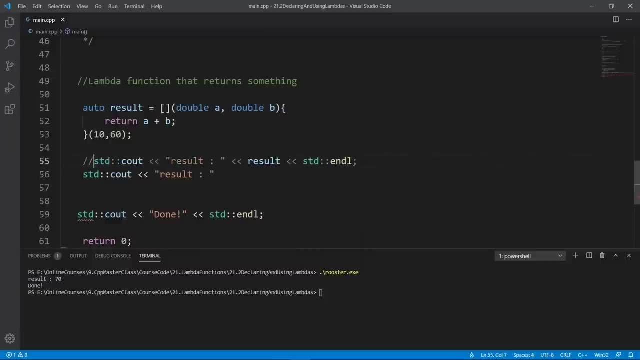 or we can even comment this out. we don't want to be confused when we look at the terminal here. we're going to comment out the first stdc out statement here and we're going to say std endl here and put in a placeholder for our lambda function and we're going to paste it in. 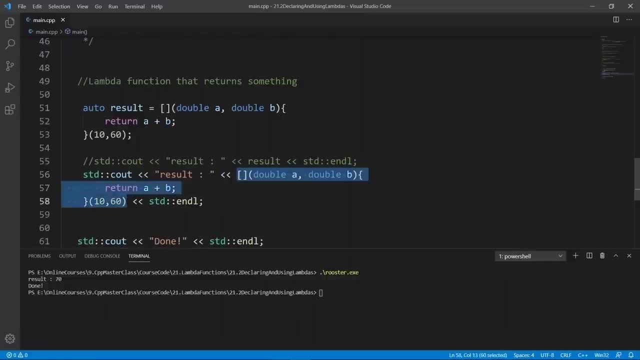 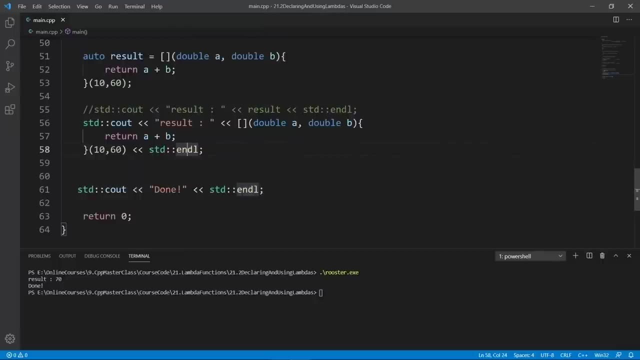 if we do something like this again, this entire lambda function thing is going to return the sum and that's what we're going to print. i realize this syntax is really cryptic, but it is going to work. let's try and build our program here. the world is good, so we can. 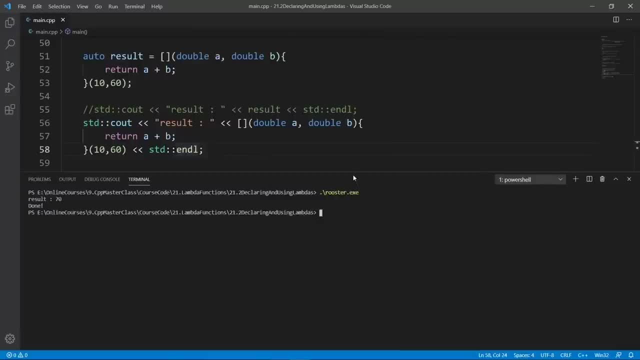 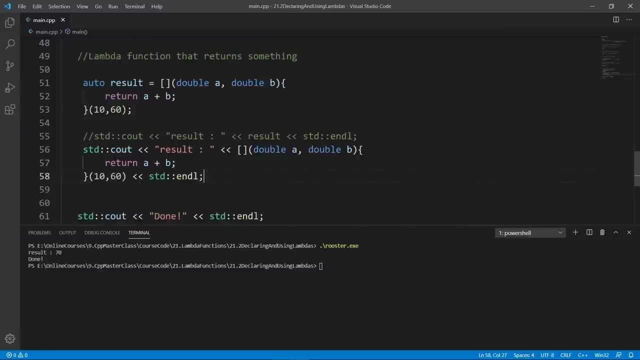 clear and run rooster. we're going to see that result is 70, and this is coming from our call here, which is nested inside our stdc out statement. you can do this if you want. another thing you can do, as we have seen before, is give your lambda function a name and call it repetitively so. 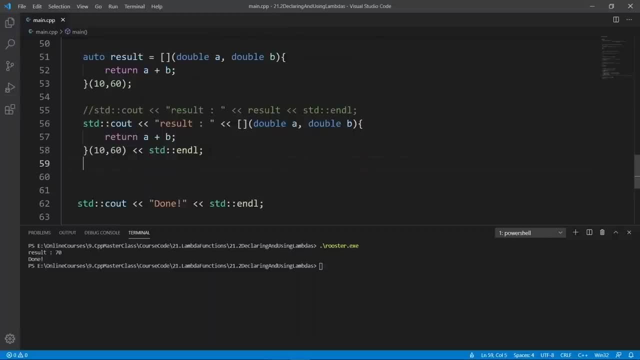 for example, we can try and comment out what we have here and set up another lambda function, because we don't want to confuse you again. so we're going to grab our lambda function here, we're going to copy it, because we don't want to type this a thousand times and we don't want to. 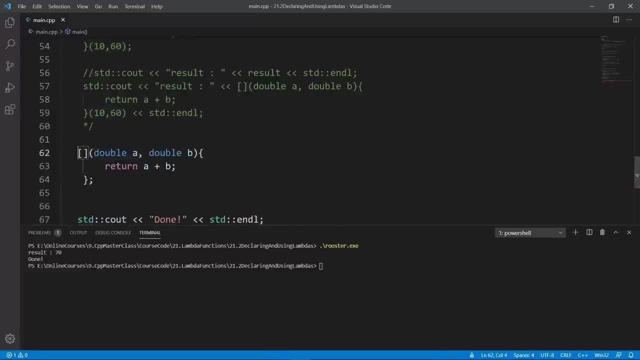 call this lambda function directly. instead, we want to give it a name and we're going to say auto funk 2 and we're going to assign our lambda function type to funk 1.. now that we have this, we can say auto result 1, for example, and we can say funk, and we can pass in whatever we want. let's. 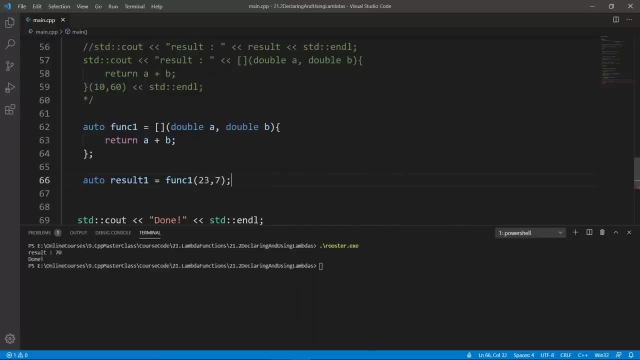 put in 23 and a 7 and this is going to add up 23 and 7.. we're going to grab the result and we're going to assign that to result 1.. if we go down and say auto, for example, result 2 and say, for example, funk 1, and say 9 and 45, why not? and go down and 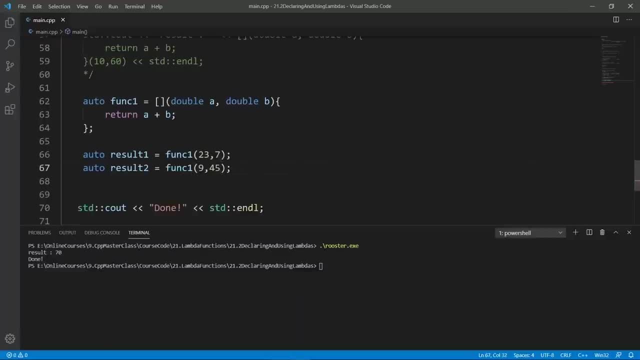 print out these result variables. we're going to see the sums printed out and again, the message is that we can use this handle to call our lambda function multiple times. so let's go down and print these out. we're going to say result 1 and we're going to say result 1. here we're going. 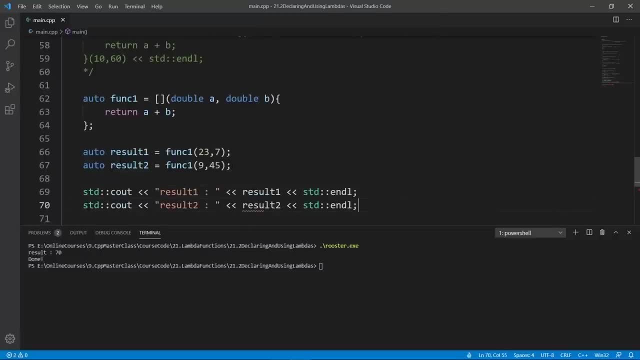 to go down and say result 2 and we're going to print that out and we can even call this lambda function directly and put that in stdc out here. so let's say that we're going to say result 3, for example, or direct call. i think this is descriptive enough. so we're. 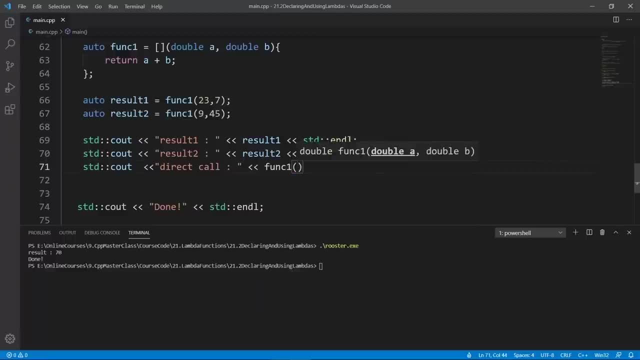 going to say funk 1, the name of our lambda function or the handle to the lambda function, and we can put in a 5 and a 2, for example, and we're going to see this print out the result. if we build our program, let's do that with gcc, the build is going to be. 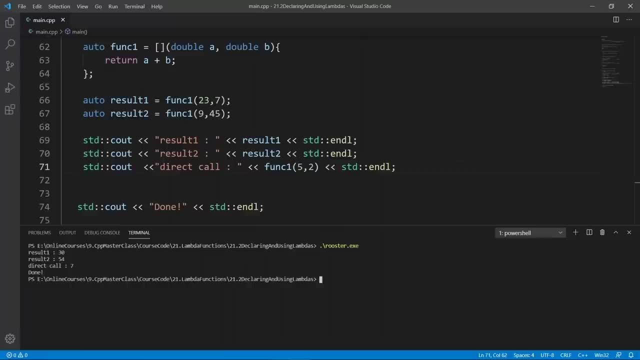 good, we can clear and run rooster. we're going to have result: 1 is 30, which is 23 and 7, so the sum is 30.. the second one should say 54 because that's the sum, and the third one should say 7 because 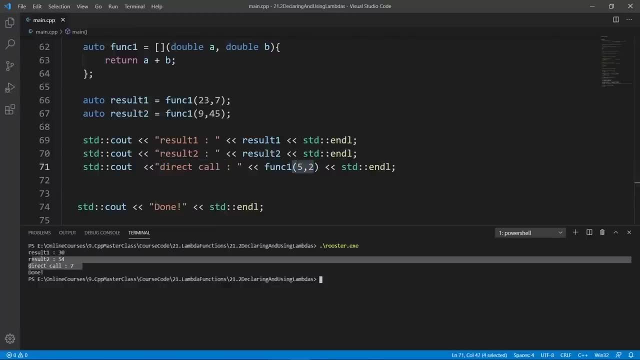 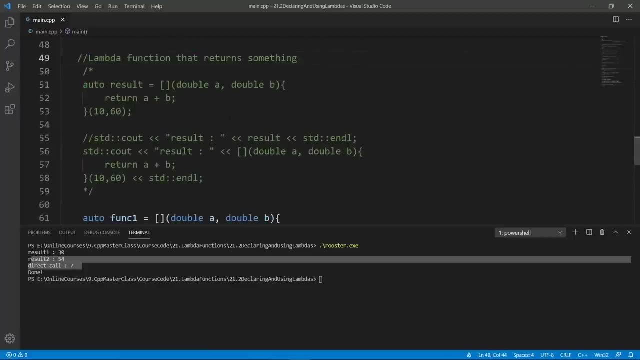 that's the sum of 5 and 2, and it is what we have here, and after that we're going to see that our program is done. this is how you can set up a lambda function that returns something, and we have seen many ways we can work with us. let's go. 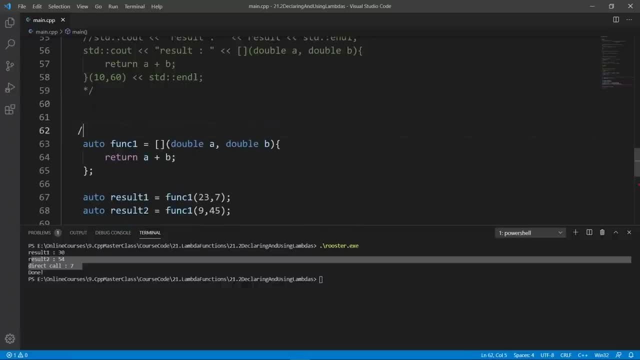 this out, because there is one more thing i want you to see, and that's a lambda function whose return type is specified explicitly. okay, we are going to reuse the same lambda function we have been using all along and we're going to copy that and we're going to go down and put it down here. 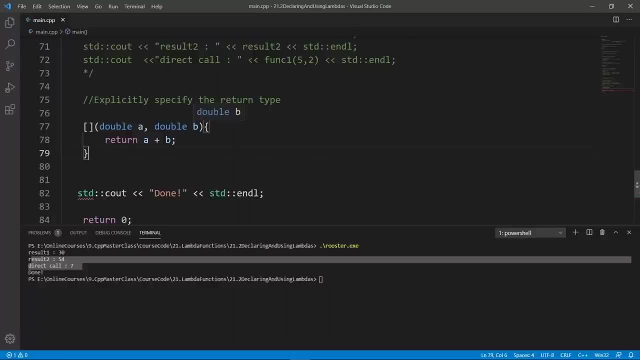 and now we want to specify the return type as double. the way we do that, we go after our parameter list and we put in a dash symbol and we put in a greater than symbol, and then we're going to specify the return type of our lambda function. let's say that we want our 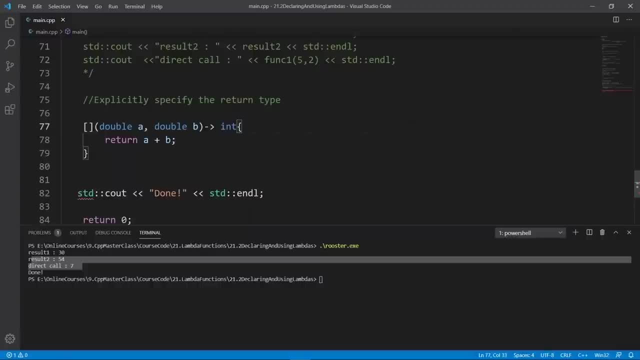 return type to be nt. this is how we say it now. our function here is going to return nt, regardless of the types that we put in. so what the compiler is going to do when we call this lambda function: it is going to take the parameters, it is going to add them up. for example, now they are double. 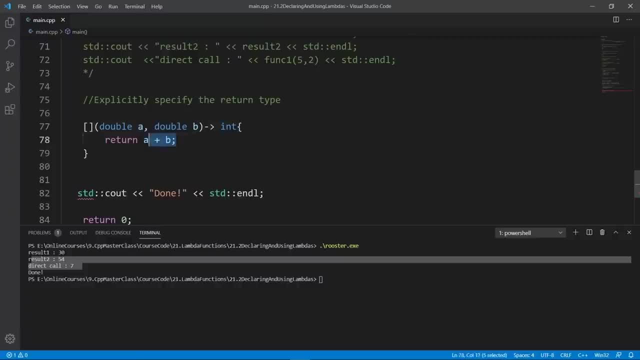 so it's going to add a and b as double. it's going to produce a double variable return it. you notice that now we have forced our lambda function to really return a specific type here, before the return type was deduced from the operation that we did here and before we were. 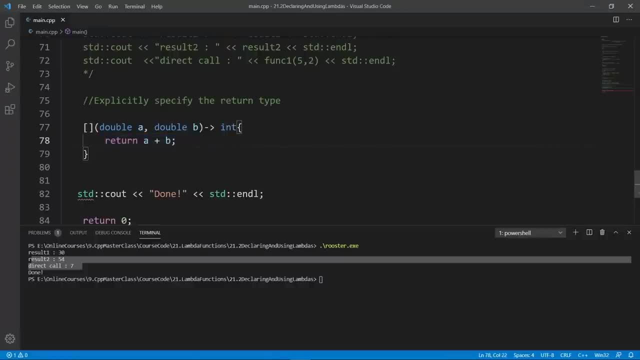 returning double, because that's what the compiler was deducing for a and b here. to really drive the point home, let's assign this lambda function to funk one or funk three. let's do that. we're going to set up a function called funk three and this is a lambda function that is going to explicitly. 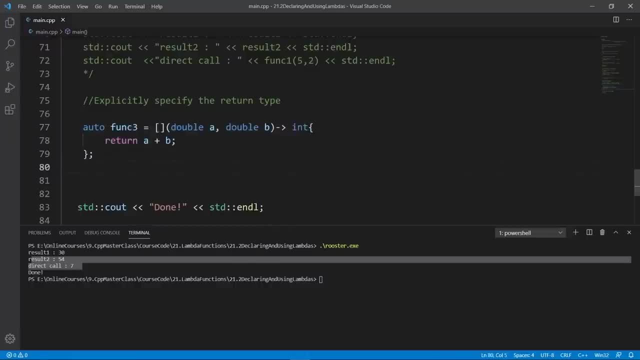 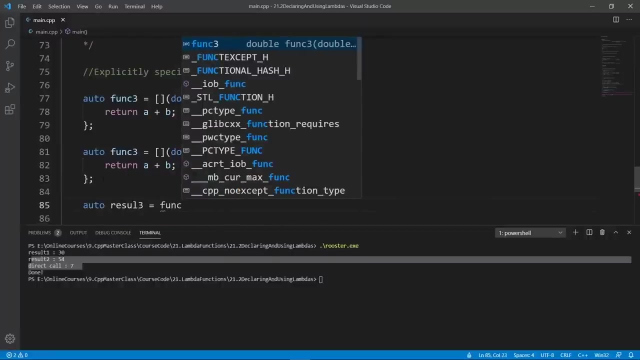 return and and we're going to set up another one which is going to deduce the return type. we're not going to specify the return type explicitly, so we're going to take out our return type here, let's do that. and we're going to go down and say auto result 3 and we're going to say funk 3. 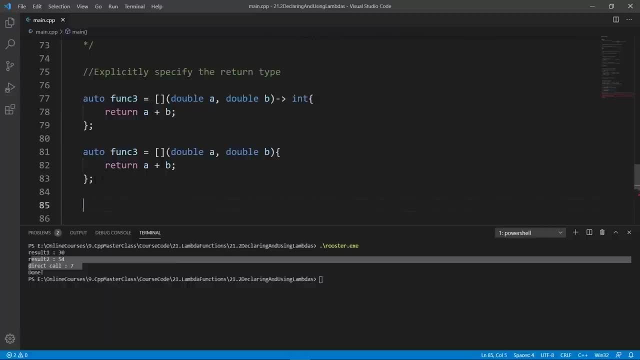 and add up two double variables. let's set up these variables explicitly so that you read the function, see what is happening. so we're going to say int a and put in a 6.9- why not? and let's make this guy double because that's what our function here expects. and we're going to do another one do. 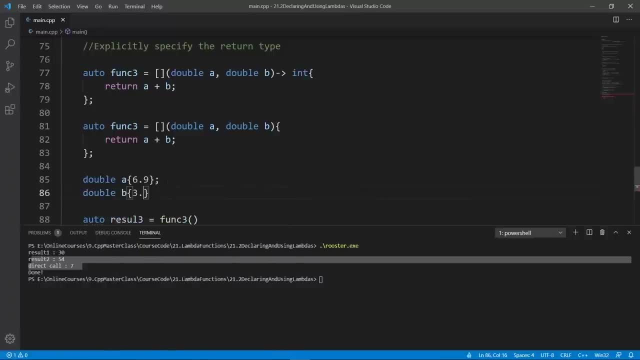 double b and we're going to put in a, 3.5, for example, and we are going to use this variables as arguments. here we're going to say a and b and we're going to say auto result four- this should be a result, and we're going to say result four and this should say result. i am making many typos. 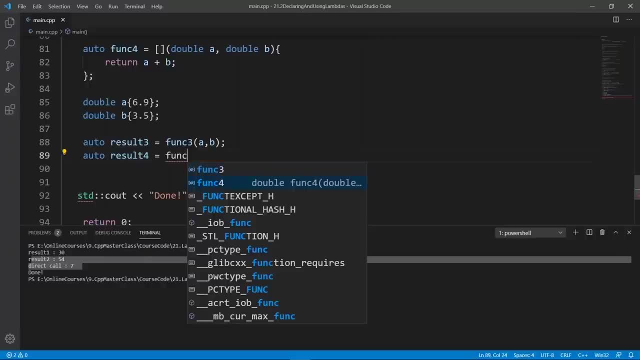 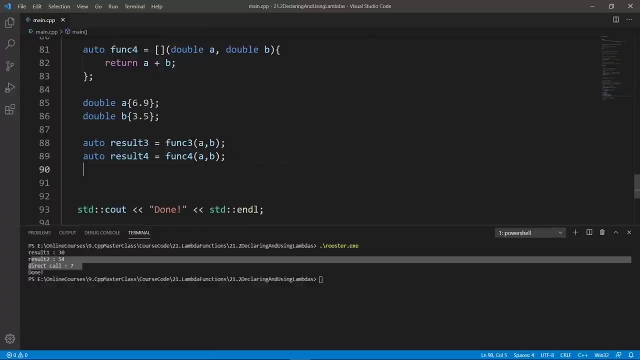 so we're going to assign our lambda function, the result of our lambda function, i should say to result four here, and we're going to pass in a and b. now we want to see the types of result 3 and result 4 here. we're going to go down and print them out. we're going to say sddc out, size of. 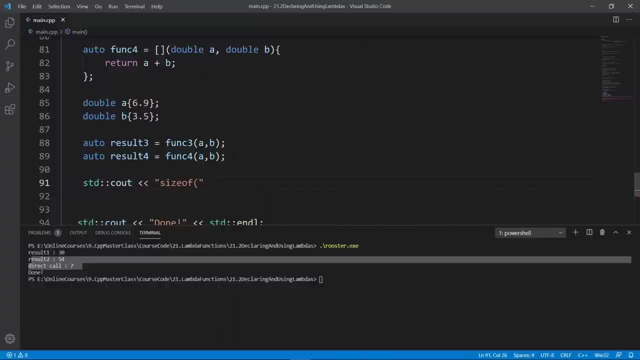 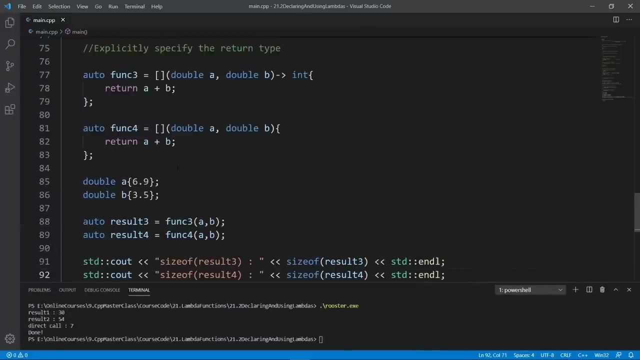 result 3 and we have to get the types of our variables. we're going to pass in result 3, we're going to say size of result 3 and we're going to go down and say size of result 4. okay, we have our code in place and what we want to see is the type that is deduced by the funk 3 lambda function here. 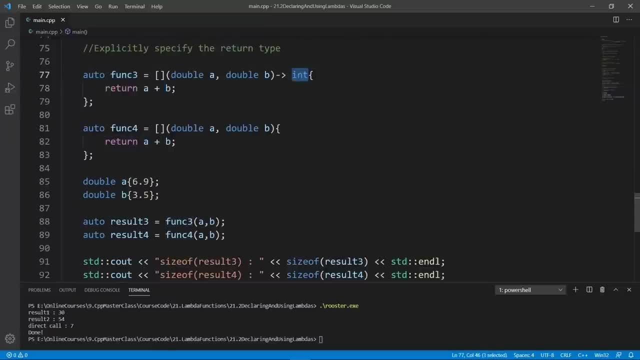 we are explicitly turning the return type into end, the parameters we pass in are going to be doubled, are going to add up a and b and the result of this is also going to be double. but the compiler is going to notice that we are returning ant explicitly here and it is going to take this. 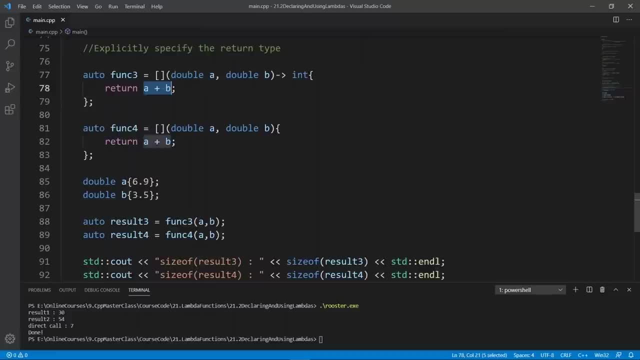 double result and transform that to ant and we're going to get- and we're going to get- the result of that assigned to func3. here for the second lambda function: here we are going to automatically deduce the return type. so what we return here is going to be a double type and we should see a. 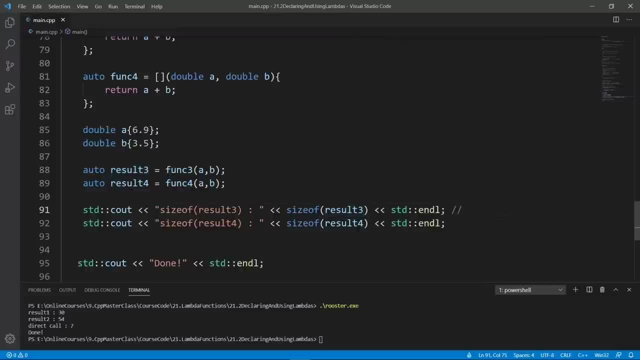 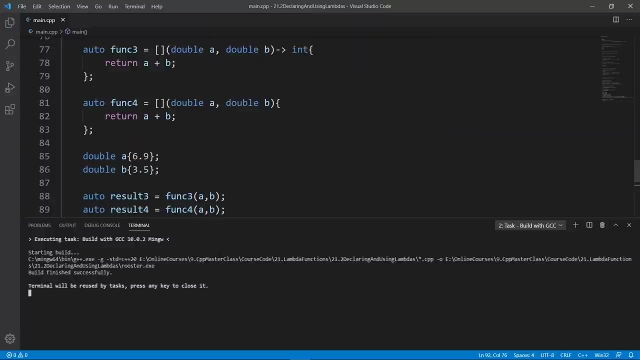 size of ant for result 3 here printed out, so we should see a 4 on my system. and for the second statement- here we should see a size of double printed out. this is one way we have to try and prove this. so let's build this program and see what we get. okay, the build is good. we can clear. 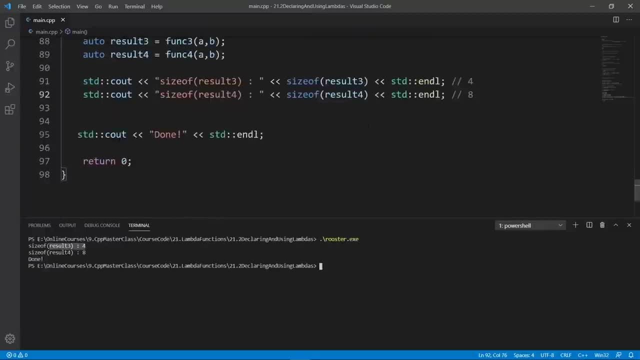 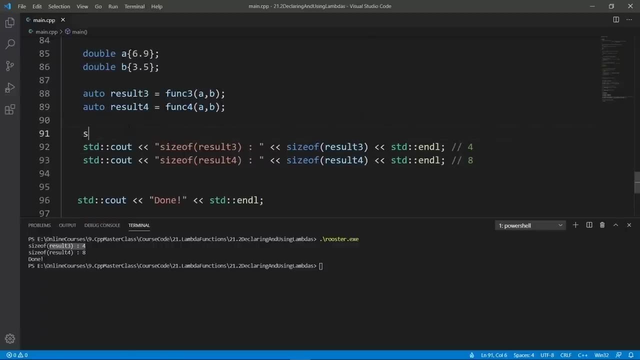 and run rooster and we're going to see that this is exactly what we expect here. you, if we want, we can even print result 3 and result 4 and see what we get. so let's do that. we are learning, so let's experiment with this a little bit. we're going to say result 3 and we should go. 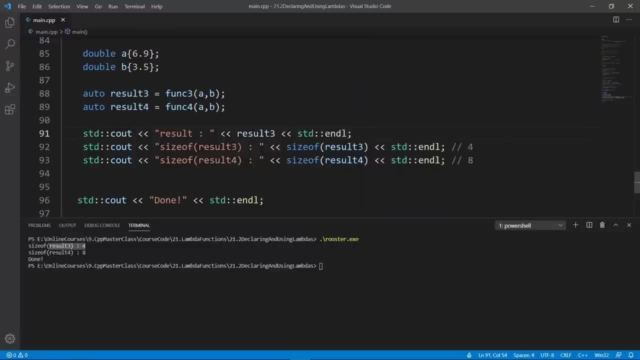 back and say result 3, if i can type endl here and we're going to go down and say sddc out result 4. okay, if we build and run this, we're going to see the results printed down. the build is good, we can clear and run rooster. 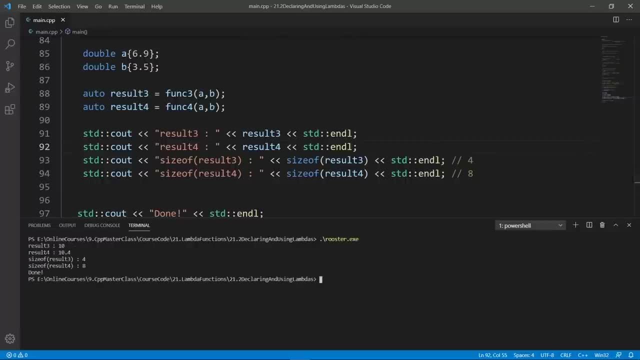 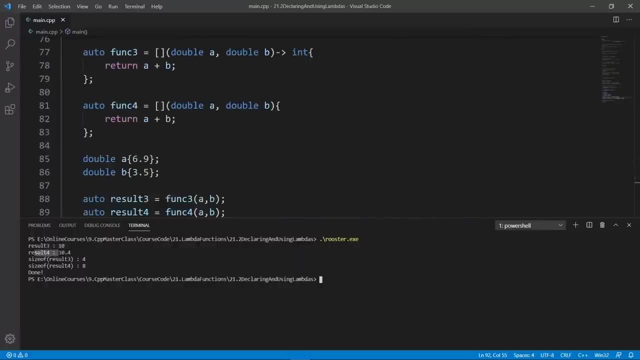 now we have: result is 10 for the first thing here, for the first lambda function, and for the second one, result is 10.4. you can see that for the first one the result was transformed from double to ant and for the second one we deduced double. so we still have our decimal point here. hopefully this. 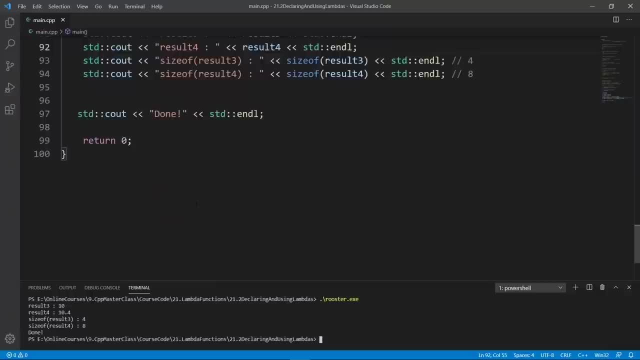 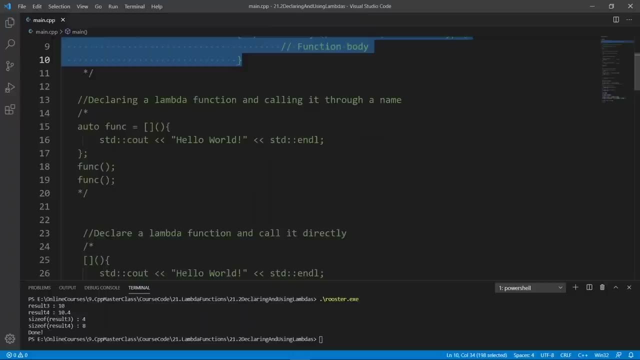 makes sense, and this is really all we set out to do in this lecture: showing you different ways you can set up your system, and we'll see you in the next lecture. bye, bye. lambda functions. we saw the syntax of setting up a lambda function. we saw that you can declare a. 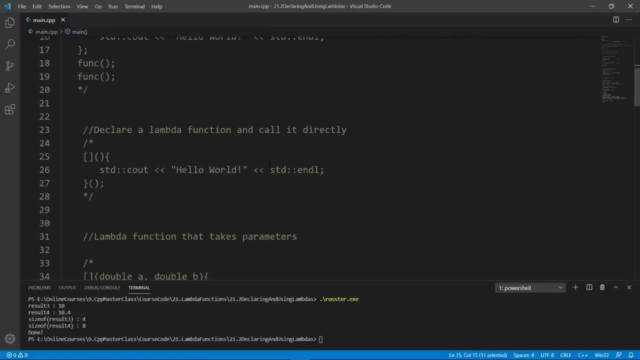 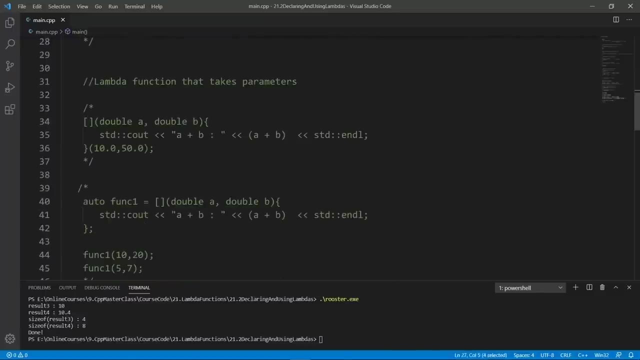 lambda function and call it through a name, like funk. here we went down and so that you can declare a lambda function and call it directly through the syntax. you see, here we saw that how we could specify parameters to our lambda function. this is the syntax and once you do this you have to. 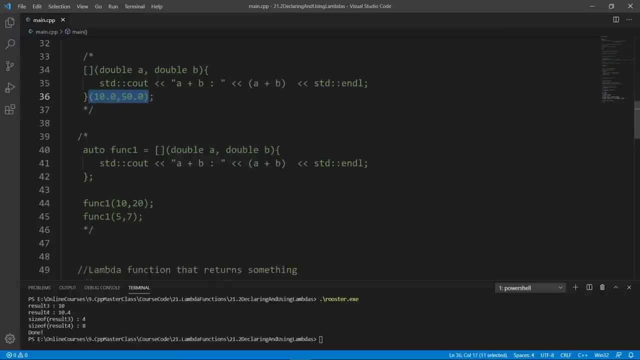 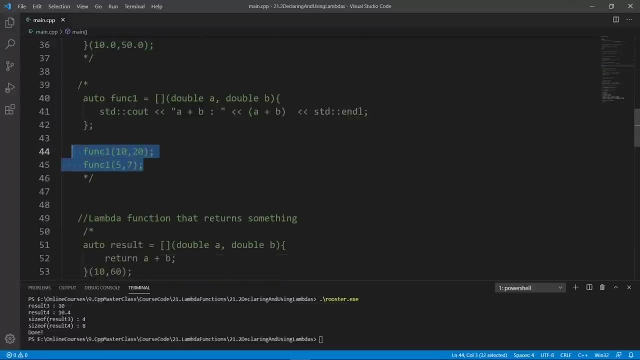 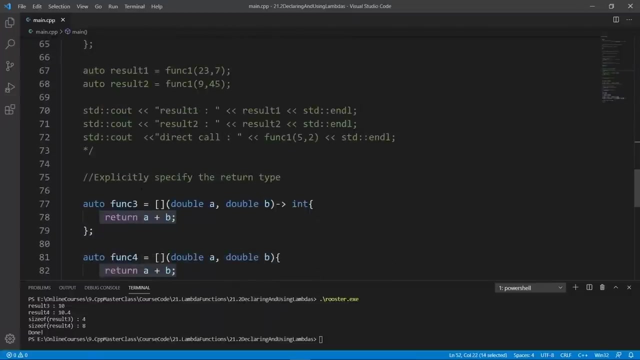 remember to call your lambda functions. with parameters, like we see here, we can even use a handle given to our lambda function and call our lambda function multiple times. after that we saw that we could return something from a lambda function and we had many chances to play with us and we finished by looking how we could. 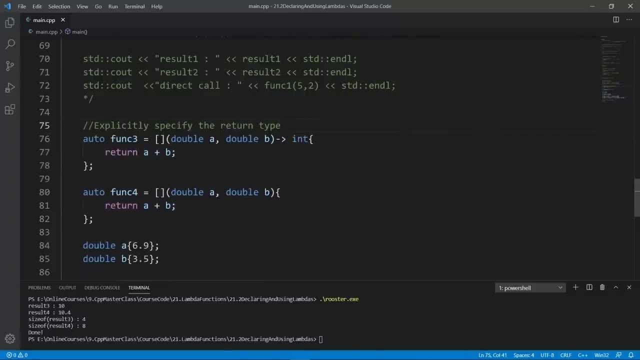 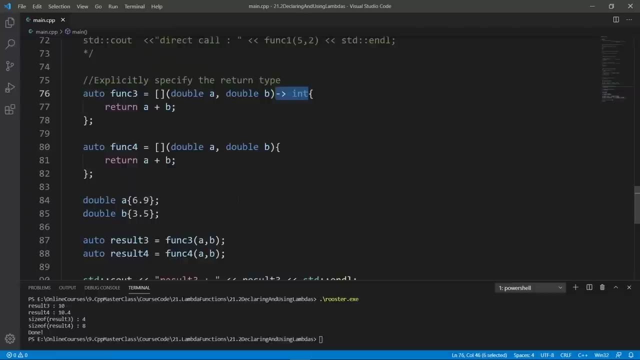 specify the return type explicitly and the syntax to do. that is what you see here. we are going to stop here in this lecture. in the next one we're going to see how we can use our capture lists here and make them do useful things. go ahead and finish the lecture. bye, bye. 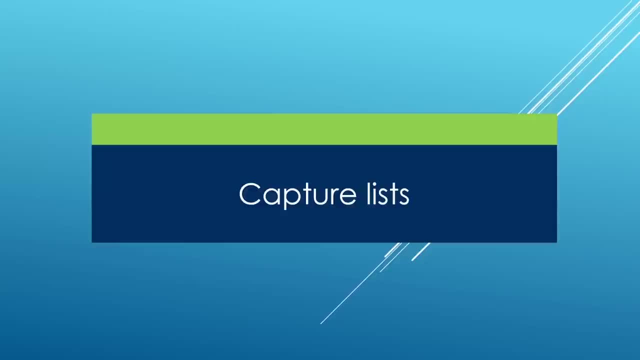 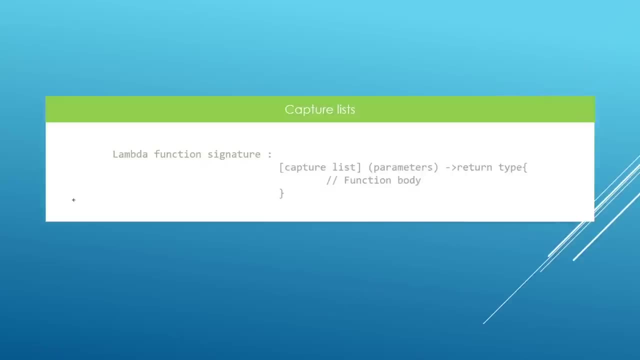 up here and meet me there. in this lecture we're going to see how we can use capture lists in our lambda functions and do some useful things. we have seen that the syntax of our lambda functions includes these angle brackets here, but we haven't really used them to do anything for what we have. 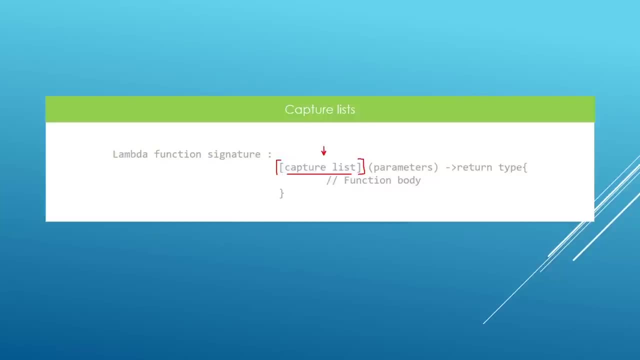 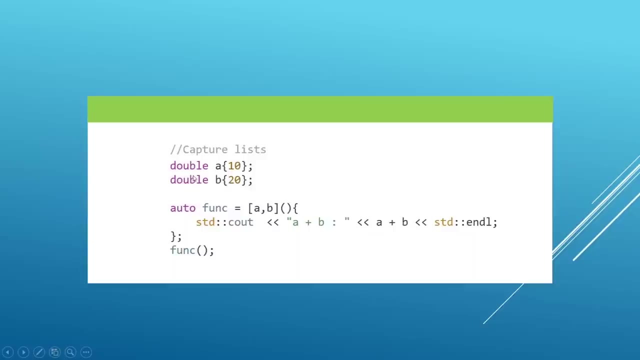 done in the last lecture. they were empty all the time. in this lecture we're going to use them. here is a simple example of how we can use our capture list. we have two variables, a and b. they are of double type and they contain these values: 10 and 20.. but 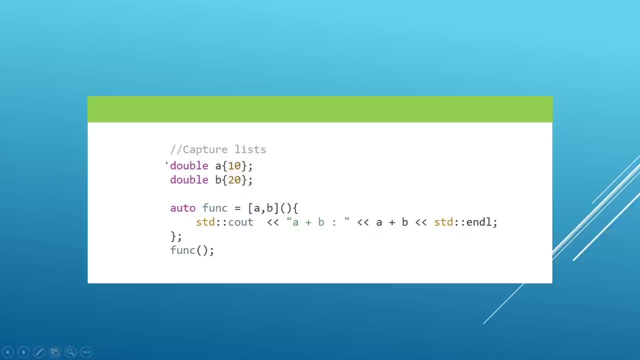 sometimes we want to use things outside the scope of the lambda function inside the lambda function here. and if you set up your lambda function with an empty capture list- suppose you don't have these two guys in- and you try to use a and b like this, you're going to get a compiler error because the 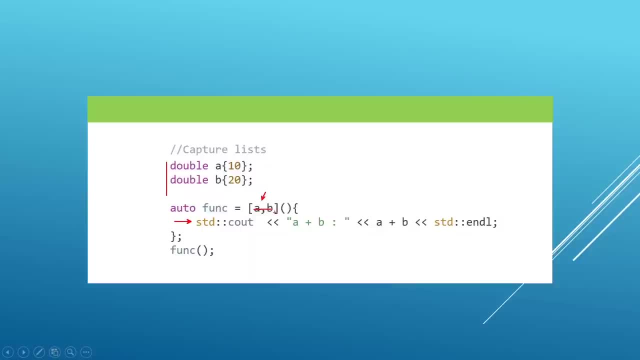 body of the lambda function doesn't have access to the output of the lambda function, so we're going to capture context here. it can only use things inside the lambda functions or things that you pass to the lambda function here, but it can't directly access things outside the lambda functions and 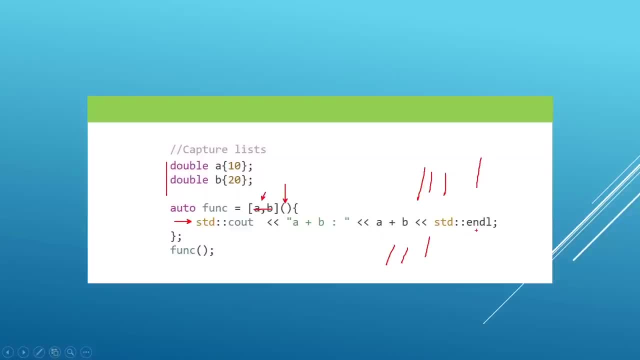 we can have access to things that are declared and defined outside the lambda function through our capture list. if you look, here we are saying a and b and this is the syntax. we have to capture these two variables, a and b, and here we are saying a and b and i can copy these variables. so we have 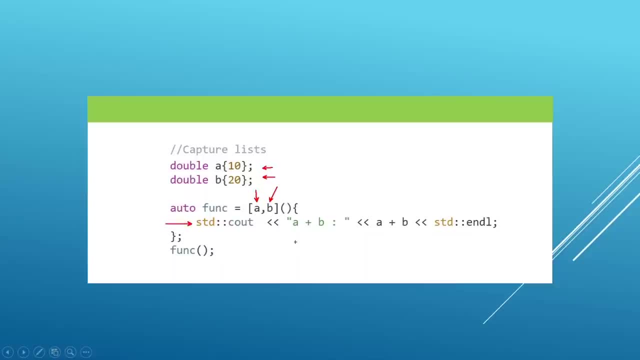 and have access to them inside our lambda function here. and this is what capture lists are really for: giving you access to things that are declared outside the scope of the lambda function, because, if you really think about it, this lambda function thing we have here is really a type, so it is its. 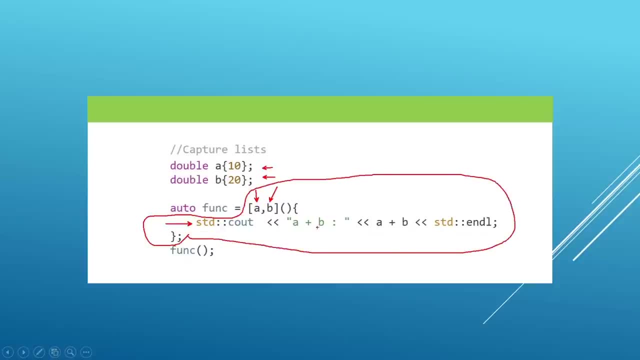 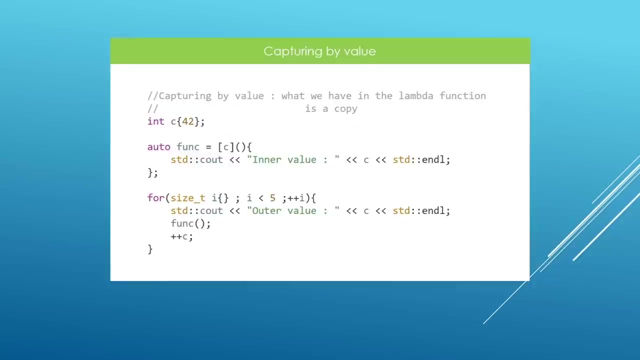 own thing that has these behaviors. well, tend so that we can call it and do things, but it doesn't really have direct access to the outside, where it was declared, and you have to give it access through the capture mechanism here. okay, now that you know this, we're going to see different ways we can use. 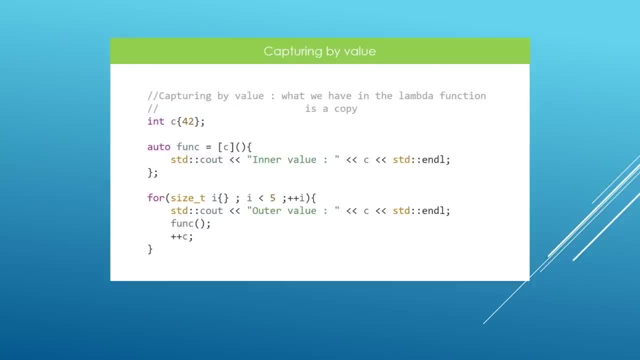 the capture mechanism. one thing we can do is capture by value, and if we capture by value, what we're going to have inside the lambda function is going to be a copy. suppose we have a variable here which is c. the value is going to be 42. as you see, here we're going to set up a lambda function and 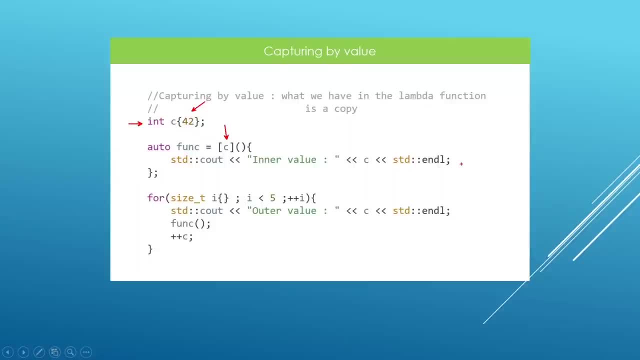 capture our c variable by value in this lambda function here and what we're going to do outside the lambda function. notice: the lambda function has a handle so we can call it. we're going to loop five times and at each iteration we're going to call our lambda function and print the inner. 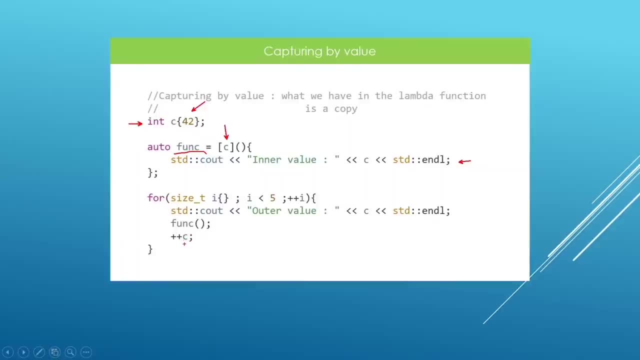 value here, but after that we're going to increment our c variable and this is going to increment the outer variable here, and what we want to see is that the changes we are doing on the outside here are picked up by the inner value that we have in our lambda function here, and i hate to break it. 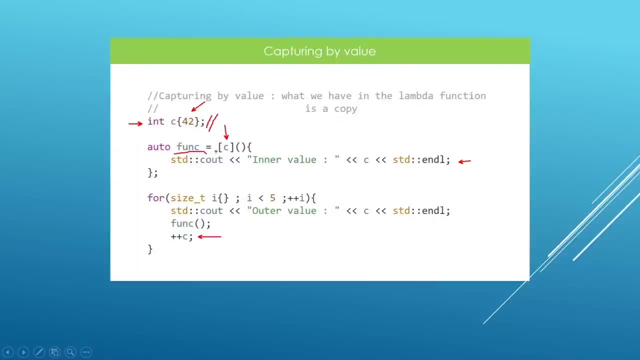 to you. this is going to not be the case, because what we have inside the lambda function is a copy of the outside variable here. so what we're going to have is for the outer value to go from 42 all the way to 47. we're going to go five times incrementing this little guy. but the thing on. 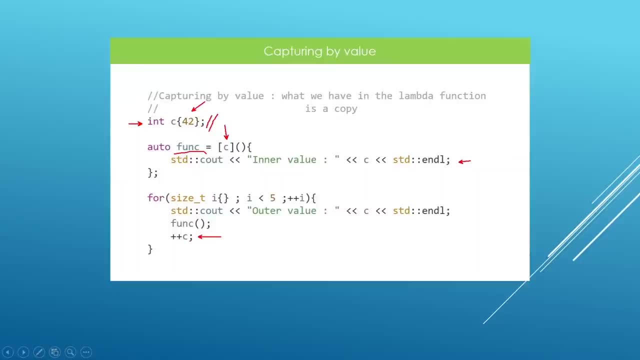 the inside is not going to change because it is a copy. the incrementation here is affected by the outside variable here, but it is not affecting the copy we have inside our lambda function. so for all these loops here, we're going to see 42 printed out and we're going to see this in a 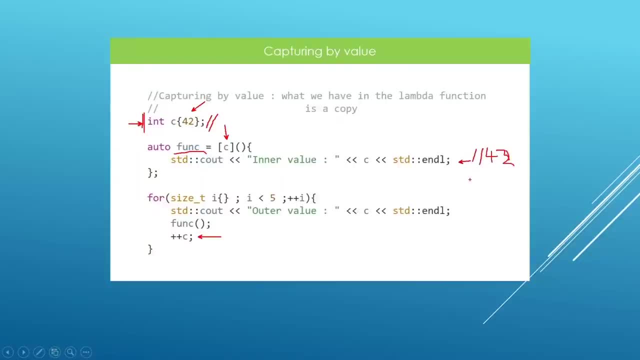 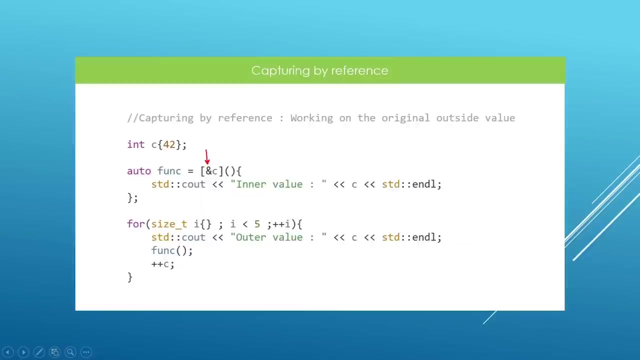 minute when we hit visual studio code, let's say 42 correctly. excuse my typing here. okay, so now you know that we can capture by a value and you know what this really means. another thing we can do is capture by reference, and the syntax to do that is to add an ampersand symbol. 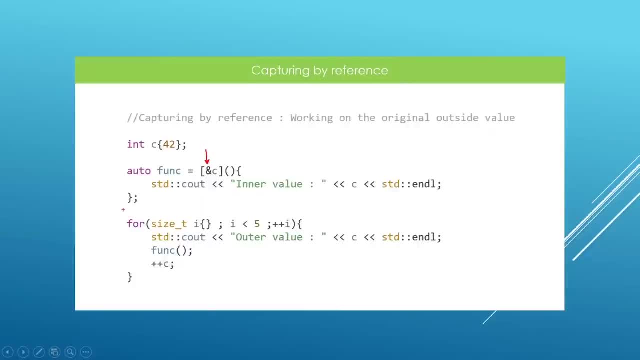 in front of the variable that we capture here. and if we do this and run the same code we run in the last lecture, we're going to see now that the changes we do on the outside are going to be picked up by the inner side of our lambda function because we are capturing by reference what we have. 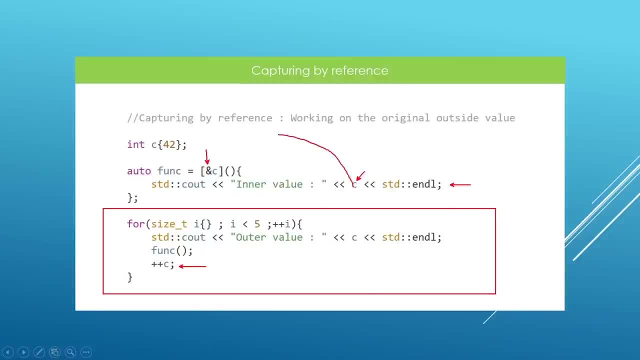 inside. our lambda function. here is a true reference to the outside variable here and we're going to see that now the outside and the inside are going to be incrementing together and we're going to have 43, 42, 44 and things like that printed out on the console. okay, this is really all i have to share. 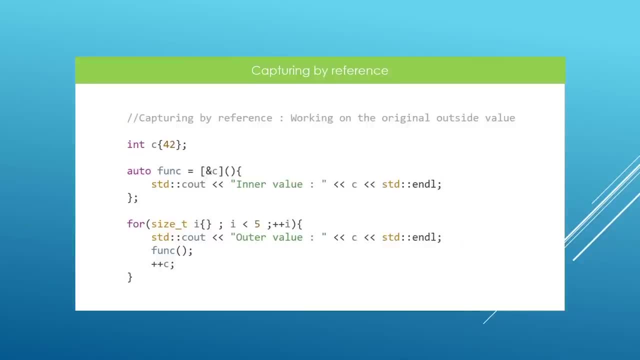 with you in this lecture, showing you how you can use your capture lists and that you can capture either by value or by reference. we're going to head over to visual studio code and play with this a little more. okay, here we are in our working folder. the current project is capture lists. we're 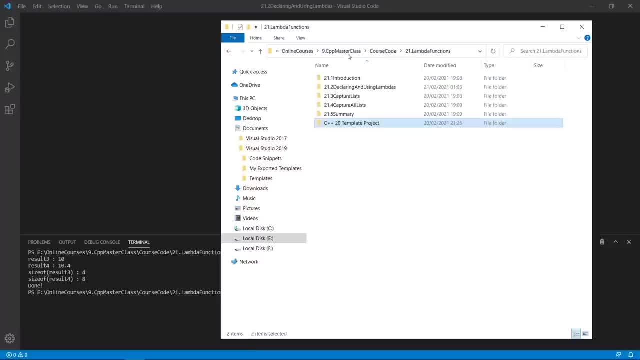 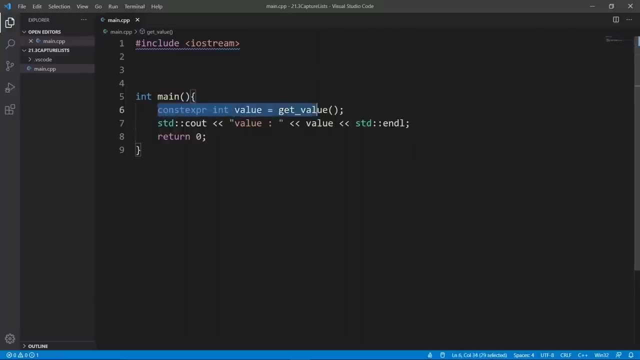 going to grab our template files pretty quick and we're going to put them in place. we're going to put them in the current project and we're going to open this guy in visual studio code by dragging and dropping in place here and we're going to open our main cpp file. clean it up a little bit and 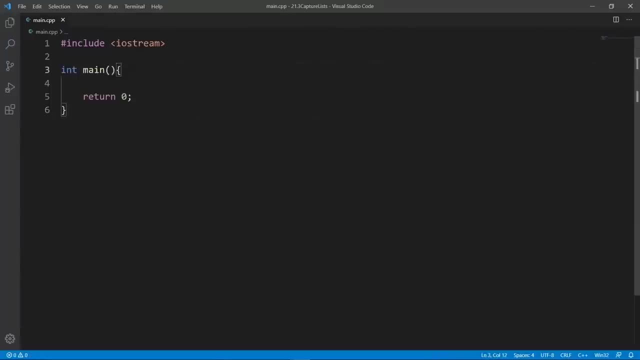 close the left pane here. what we want to do in here is learn a little more about capture lists, and we're going to put in a piece of code to play with just that. we have two variables, a and 10, here, and we have our lambda function set up. 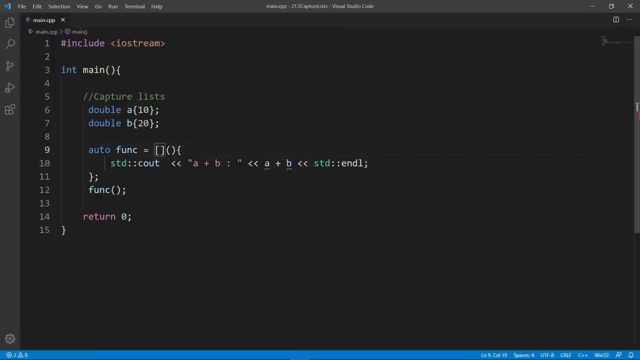 and let's take out our capture list so that you can see the compiler error we see if we try to use them as is here. so we have our two variables and we have a lambda function set up here and inside the lambda function, notice that we are trying to access variables that have 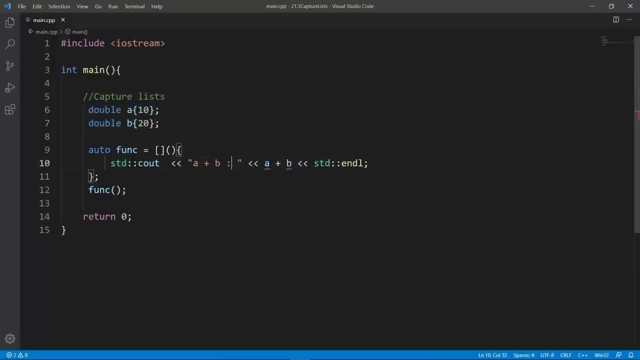 been declared on the outside of the lambda function here and by default. if we try to do this, we're going to get a compiler error because these two variables don't exist in the scope of the lambda function here. let's bring up a terminal and see what visual studio code is saying about this. 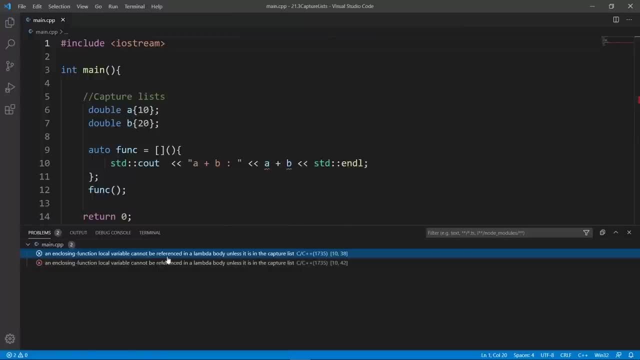 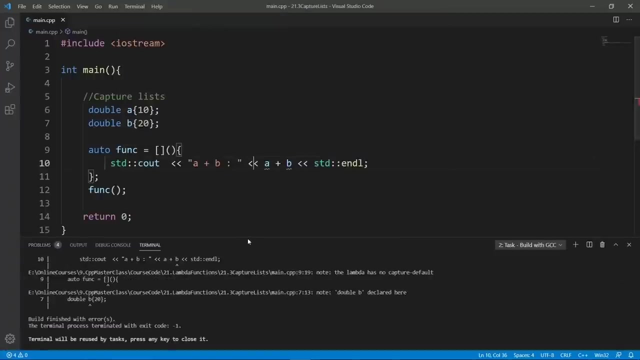 and it is going to say: an enclosing function local variable cannot be referenced in a lambda body unless it is in the capture list, and you see that this is really descriptive. okay, we have sent this error, but we want to see what the compiler says about this. we're going to pass this through gcc and we should get a similar error. it is going to say: a is not. 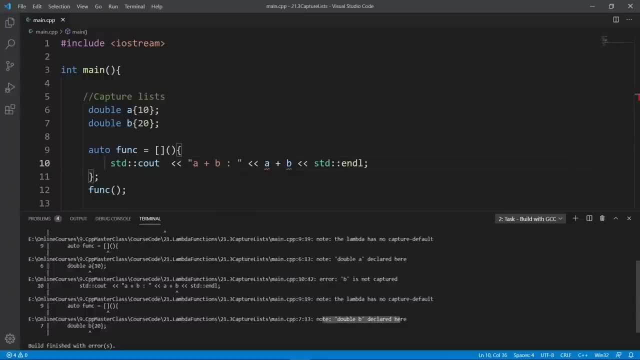 captured and it is going to go down here and say b is not captured here, and this is the error. we are trying to use outside variables in our lambda function, but to really do that we need to capture a and b and the syntax to capture our variables is to put them inside our angle. 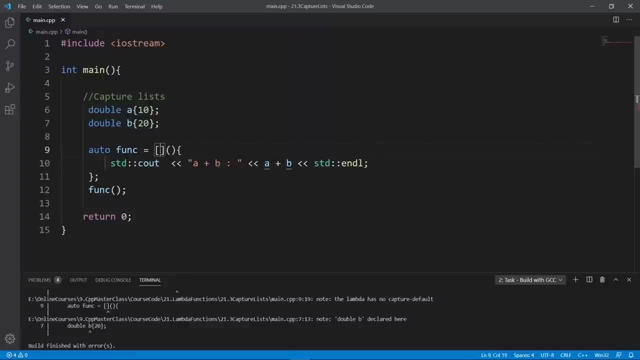 brackets here with a comma separated list of the variables that we want to capture. so we're going to say a comma b, because that's what we want to capture here and the moment we do that, visual studio code should be happy. it is not happy. i think we need to compile this for it. 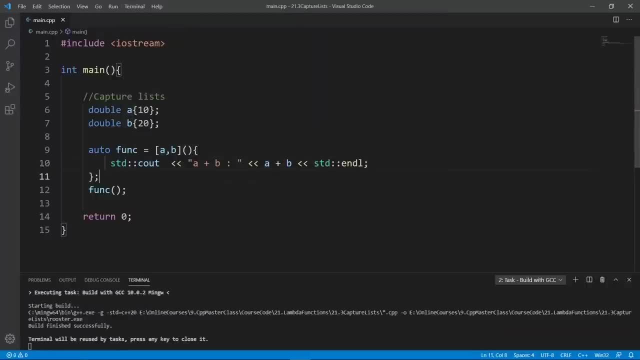 to be happy. so let's do that. and you see, now our variables are being captured and we are summing them up and we are printing the result of adding them up here by calling the function through a handle we have set up here. hopefully this is really making sense. let's build the program again. 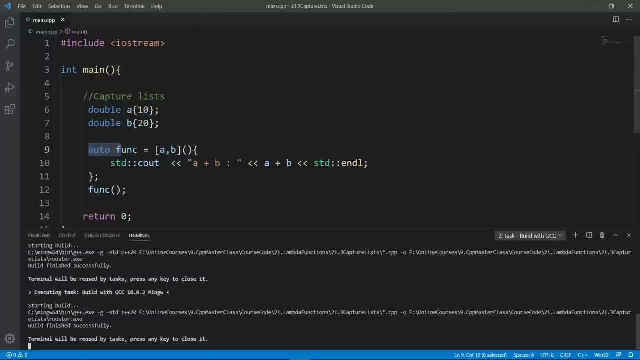 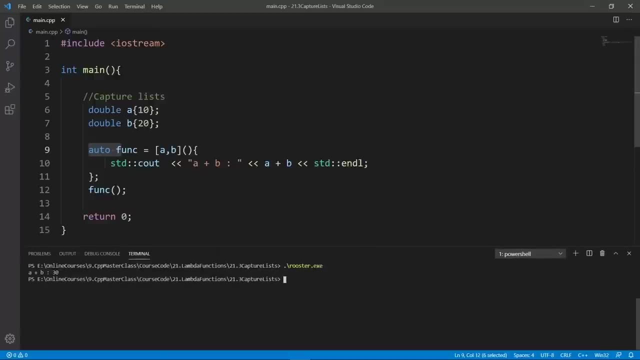 so let's use the gcc. you're going to see that the world is good, we can clear and run rooster. we should see a plus b is 30, but the values are getting inside the lambda function through our capture list. they are not going through the parameter list here. this is really something you need to be aware of now that. 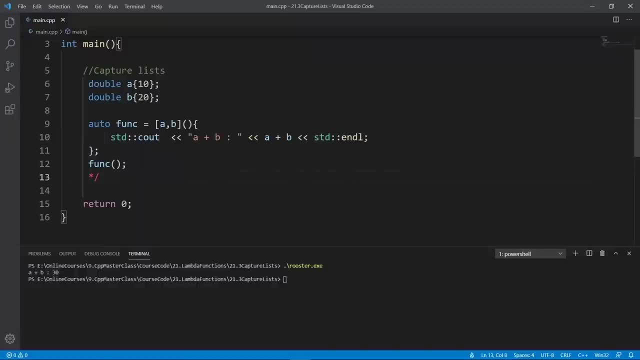 you know how capture lists work. let's see that you can capture either by value or by reference, and we're going to see what that means exactly. i going to go down here and put in a piece of code to play with capturing by value. okay, let's do that. 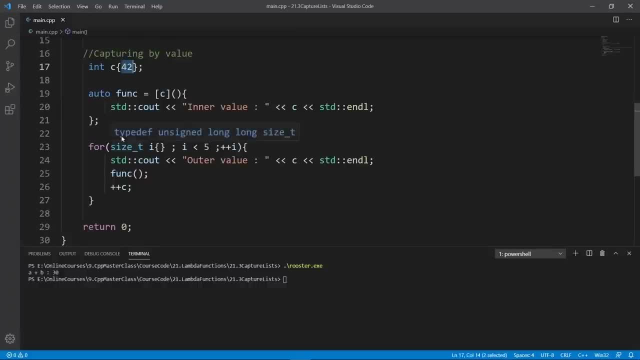 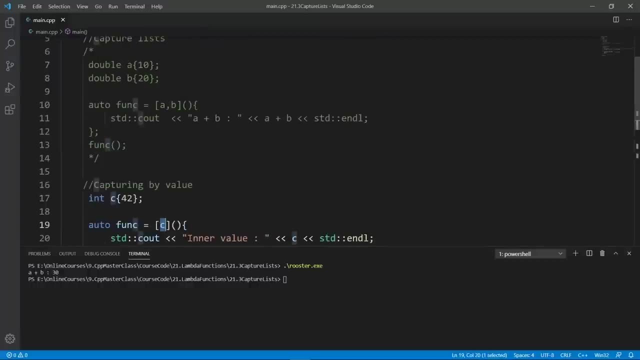 we have a variable called c, the value is 42 and we set up a lambda function which is going to capture c with this syntax here and this is the default syntax we saw, like we did on top here. so we are going to be capturing like this and if we do this, we're going to be capturing by value, the meaning. 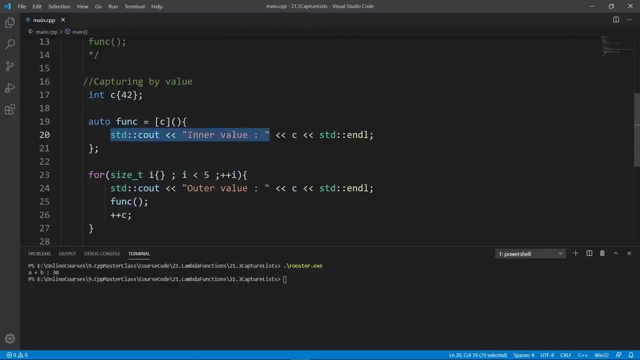 of that is that what we have inside our lambda function is not going to be the original value here. it is going to be a copy of what we have there. what we can do here is use this length in a loop and really prove this. so we're going to loop five times, from zero all the way to four. 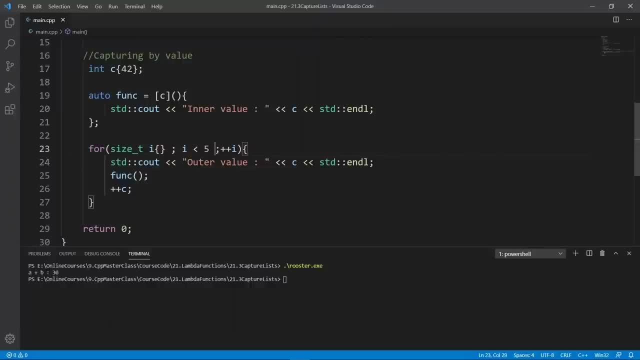 because this is going to go until i is no longer less than five, and inside we're going to paint the outer value, which is going to be the c here. after that we're going to go um our lambda function, which is going to print the inner value in the lambda function. 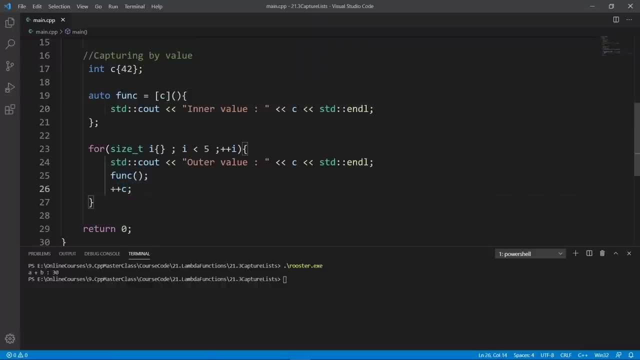 and we're going to see that the incrementation we do on the outside, which is going to affect the outer value here, is going to be visible inside the lambda function here and that's not going to be the case. the change we do here is not going to be picked up by the lambda function here. 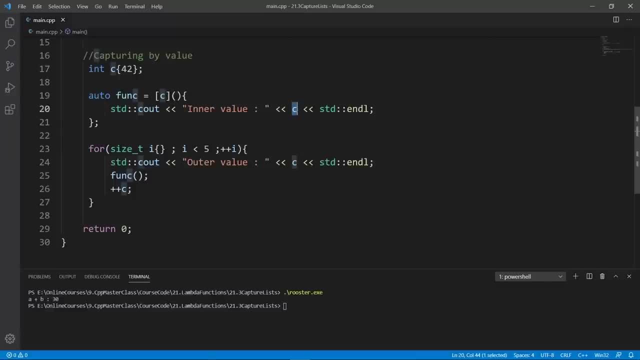 because what we have inside is a copy. so what we're going to see is for the outer value to go from 42, 43, 43, 45, and it is going to go until we hit the end of this loop here, but the inside value is not going to change because the change we're doing here is not going to affect the copy. that 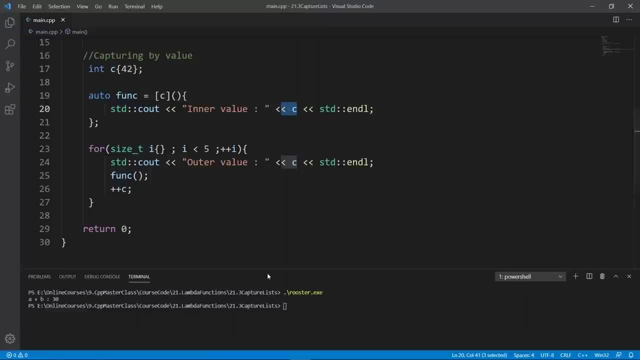 we have in our lambda function here. hopefully this makes sense and again, if you have a problem, please make sure you ask through the course platform and i will do the best i can to help you out. for now we're going to build and run this program. you. 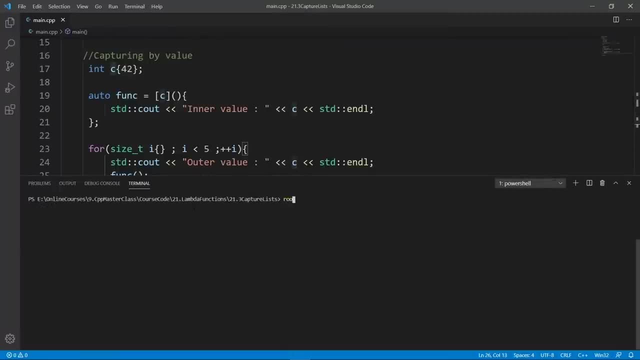 see the build is good, so let's clear and run rooster. you're going to see outer value is 43, outer value is 43. outer value is 44. outer value is 45. the outer value is changing but the inner value is staying at 42, as you see here. hopefully this proves that the outer value and the inner 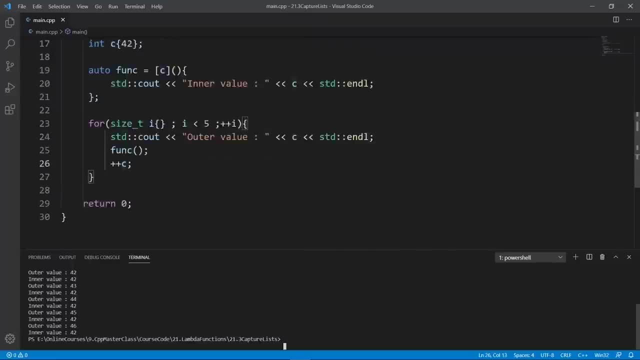 value are two different things. but we can even go further and print the addresses of the outer value and the inner value. let's do that. you're going to add that to our statement here and say the address of this guy. so we're going to say address of outer value or say address of 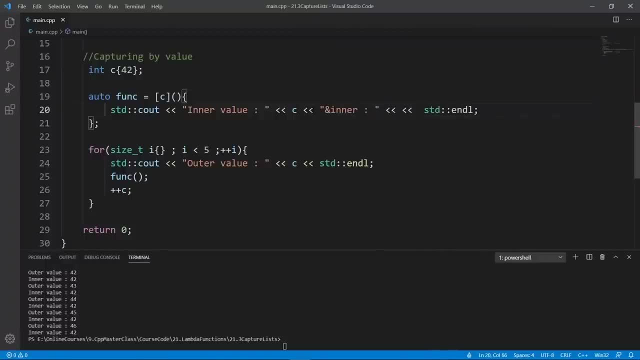 inner value. we can say it like that to really be descriptive in our terminal here. so we're going to say the address of c and on the outer value we're going to add another piece of information and say address of outer value and we're going to say the. 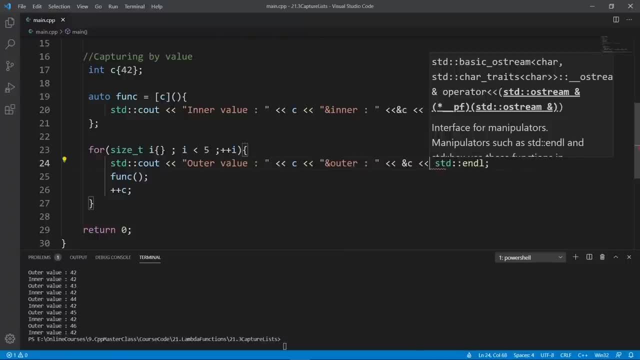 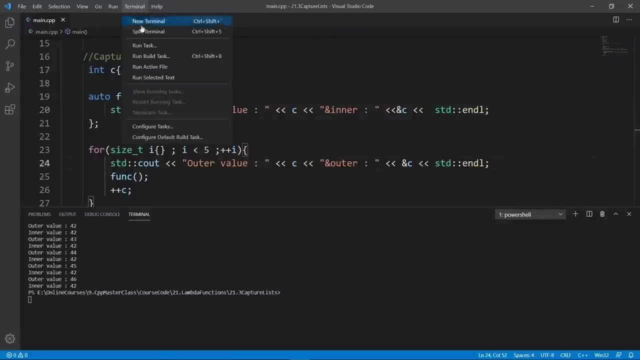 address of c and this is going to pick up the outer value that we have here and this is going to use the inner value we have in our lambda function. here let's try and build and hopefully these two addresses- the inner and outer addresses- are going to be different. that's what we want to. 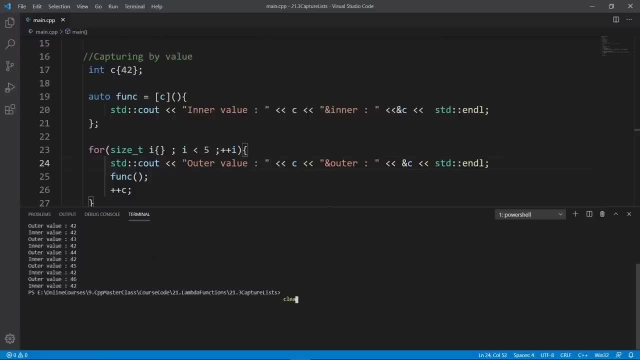 see here and really proving that what we have inside the lambda function is a copy through the capture mechanism. so let's run the program. the build was good. so the outer value, the address, is d e4. the inner value, the address, is d e0. we are proving that what we have inside our lambda 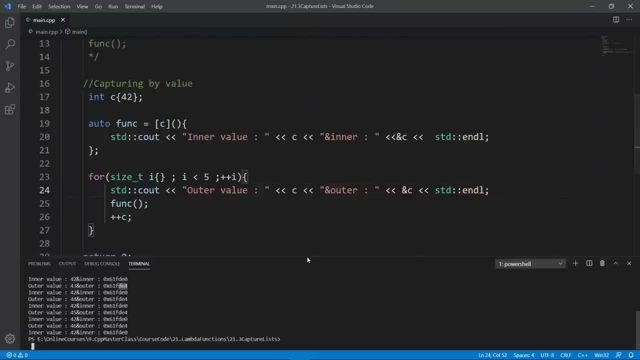 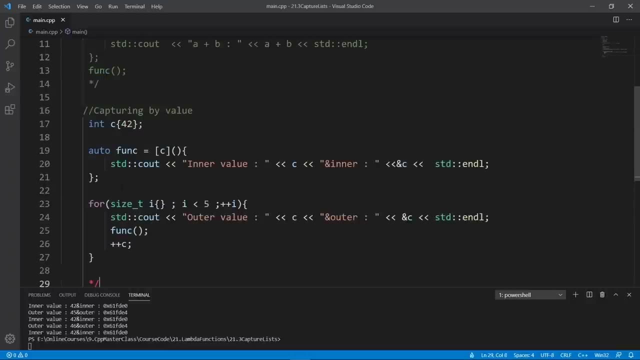 function is really a copy. so this is how you can capture by value and that's going to make a copy. but sometimes you really want to capture by reference and we're going to see how you can do that. so we're going to comment out the code to capture by value here. we're going to grab the 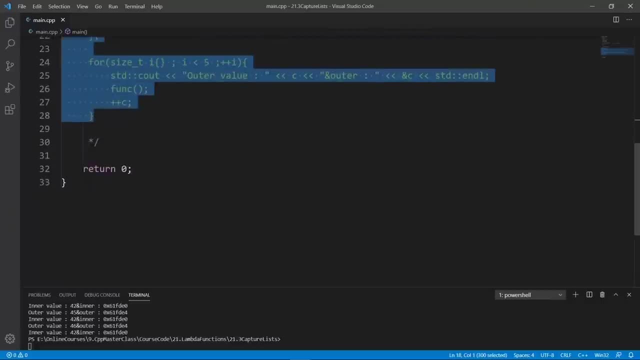 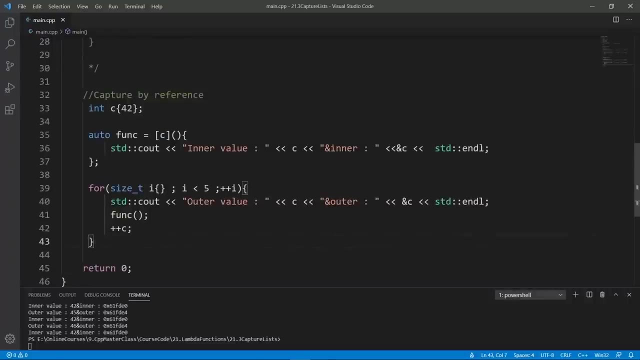 code and reuse it, because that's going to be very similar to what we had before. we're going to say: capture by reference. we're going to put in our code and we're going to change it a tiny bit. what we're going to do is add an ampersand symbol in front of our variable here that we are capturing. 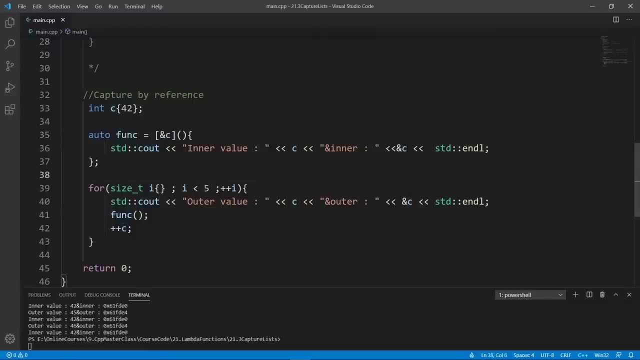 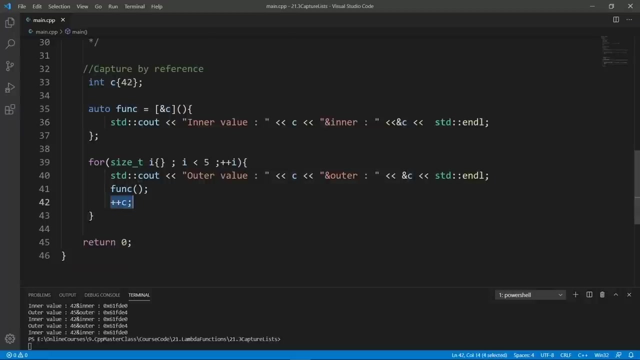 and we're going to say ampersand. the moment we do this, what we have inside the lambda function is no longer a copy. it's going to be a true reference to the outer value. here and now, the changes we do to our outer value are going to be visible inside the 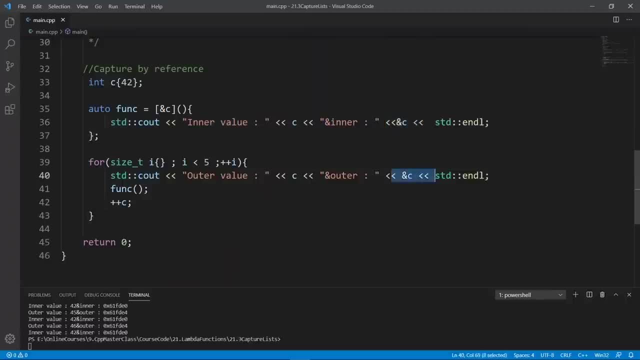 lambda function here and you're going to see the addresses to be the same. let's build and really see this. we're going to use gcc to build our program. the world is good. we can clear now and run rooster and we're going to see that the outer value. let's make sure we have some spaces. 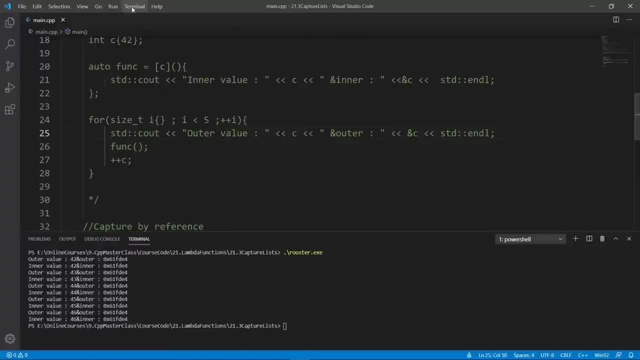 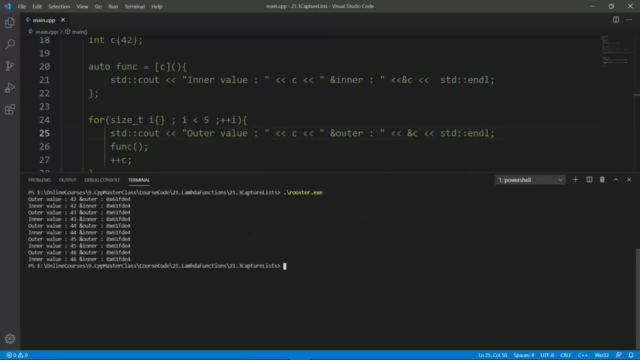 after these guys and let's go up and do that and build again, because things are really cramped together and i don't like this. so the both is good. we can clear and run rooster, so we're going to see the outer value and the inner value are changing together. 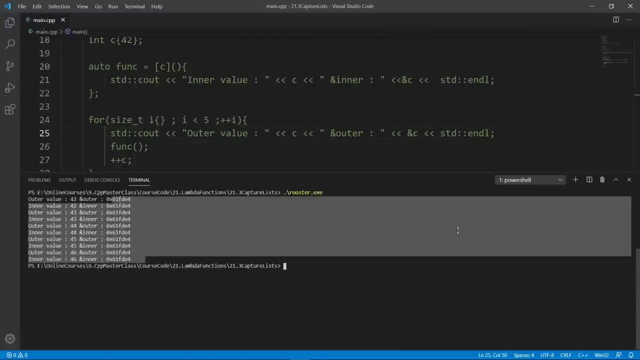 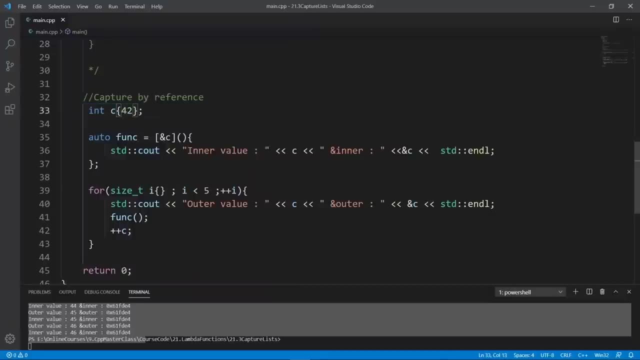 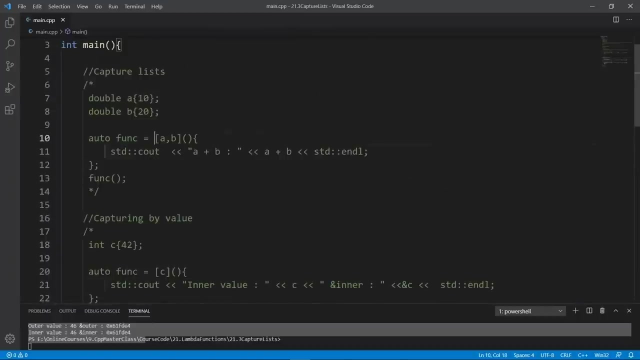 and the addresses are now the same because we have captured by reference the inner value and the outer value are referencing the same variable we have outside here. this is really all we set out to do in this lecture. i hope you found it interesting. the main idea was the. 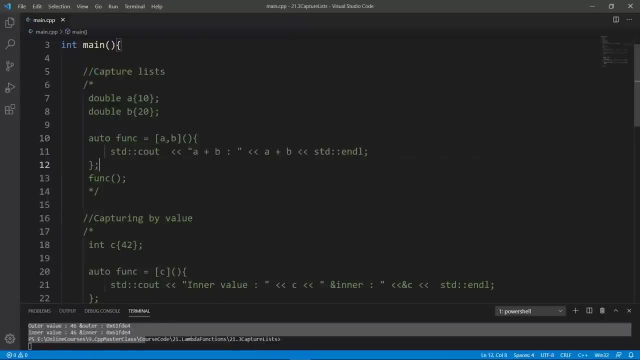 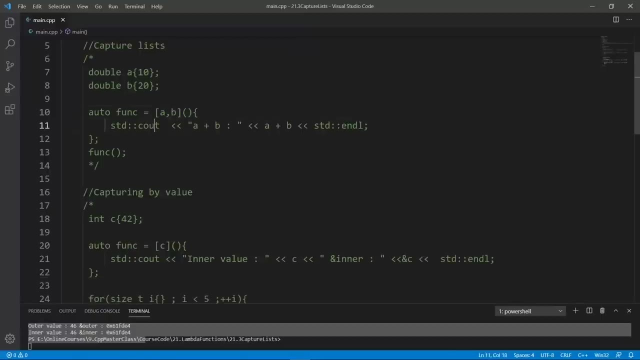 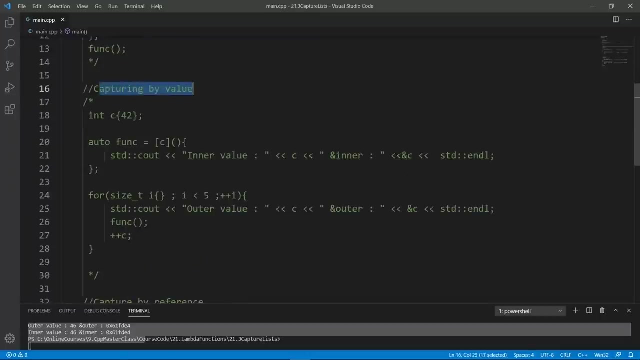 mechanism we have with our lambda functions to capture things outside the context of lambda functions. we can capture by specifying a comma separate to the list of the variables that we want to capture and we have the option to either capture by value by using the variable directly in the capture list. 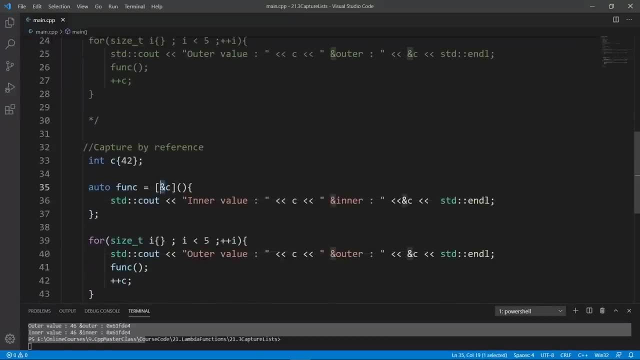 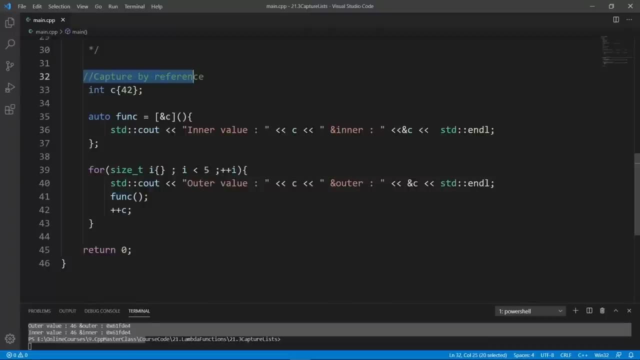 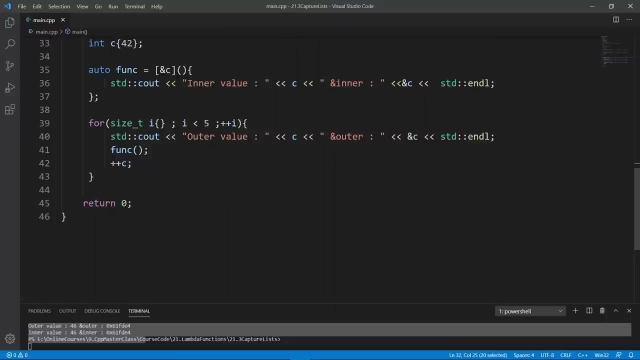 like we do here, or by prepending an uppersand symbol here and capture by reference, and you are going to have to choose whichever way you want to capture your variables. now that you know about all these options here, we are going to stop here in this lecture. in the next one we're going to see how we can. 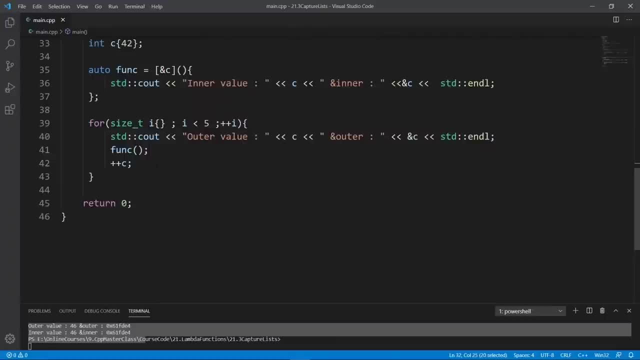 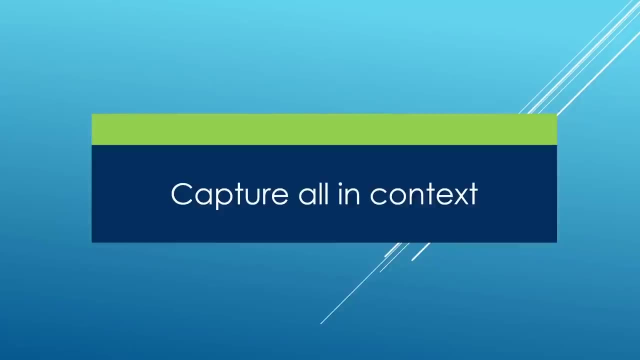 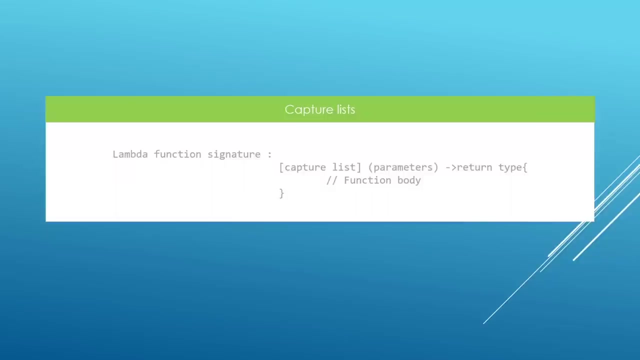 capture everything from the outside the context to the lambda function. go ahead and finish up here and meet me there. in the last lecture we saw that we could capture things outside the context of the lambda function. now we want to see that we can capture everything you can living outside the context of the lambda function. the syntax to do that is: 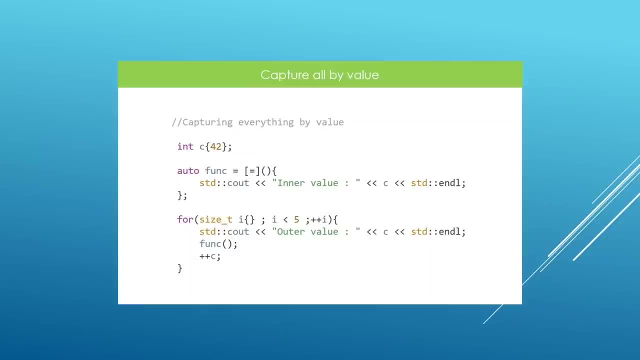 ridiculously simple. if you want to capture everything by value, you just put an equal sign in your lambda function capture list, and if you do something like this now, you're going to have access to everything outside the scope of the lambda function. for example, we can access the c variable here from the 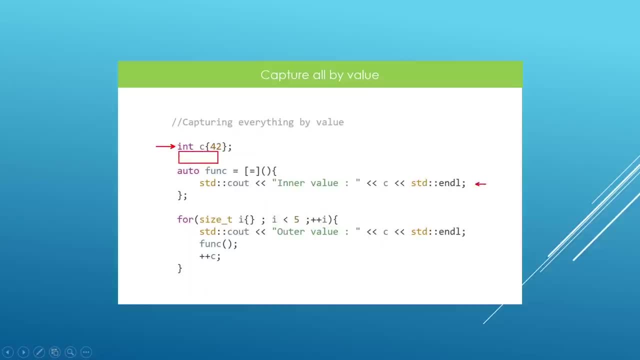 function, but if we have any more variables declared outside the scope of the lambda function, we can capture everything by value by using the lambda function in the method tower function. however, this is such a short blanket. OK, let's talk about the whole. first one, the one to keep it simple, is: 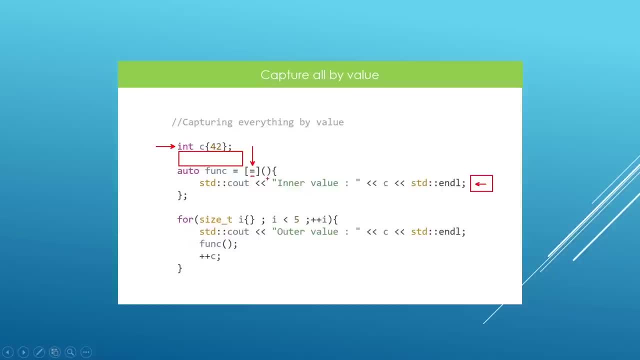 here a simple formula that is what we have for from the lambda function and that is so called the�� pets in the tupt ow, what we're doing inside the lambda function that we do here. we use it basically to get the normal values to come them inside of the 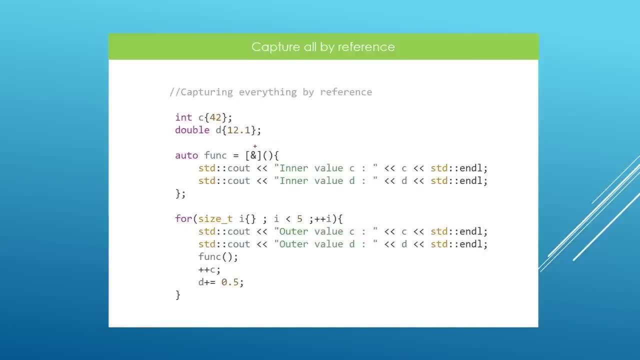 lambda function. right, so this is ourätta. that's our lambda function. so now we'll use this for our lambda function. if we get to the lambda function we will be. the syntax is really simple. all you have to do is put an ampersand symbol inside your capture list. 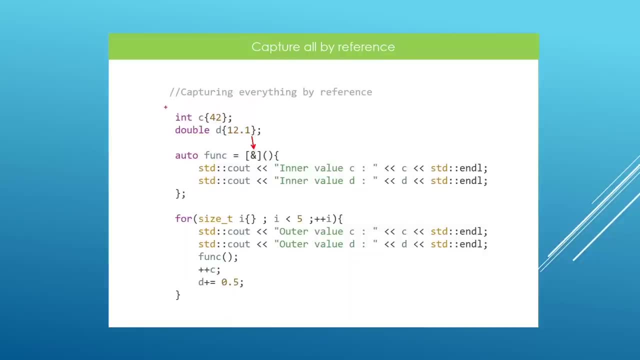 the moment you do this, you're going to have access to everything outside the context of your lambda function, but that's going to be by reference. what you have inside the lambda function are going to be true references to the outside variables and you can do pretty nasty things with them, because 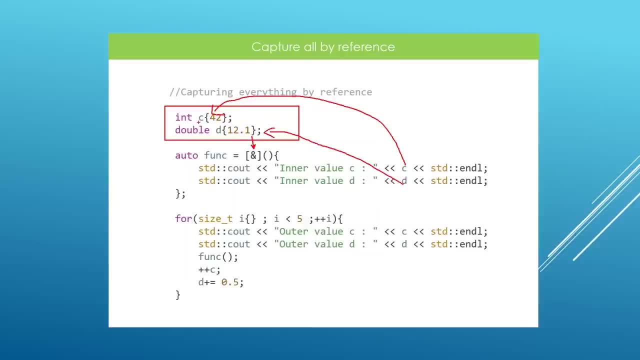 the changes you do inside the lambda function are going to be visible outside the lambda function, and any change you do from the outside is also going to be visible inside the lambda function. so if you do this, make sure this is what you want and you can use this to your advantage. okay now. 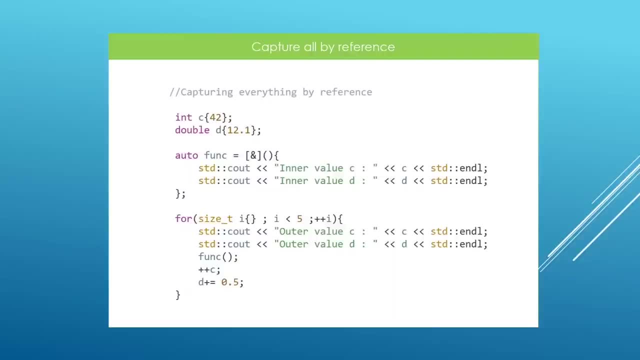 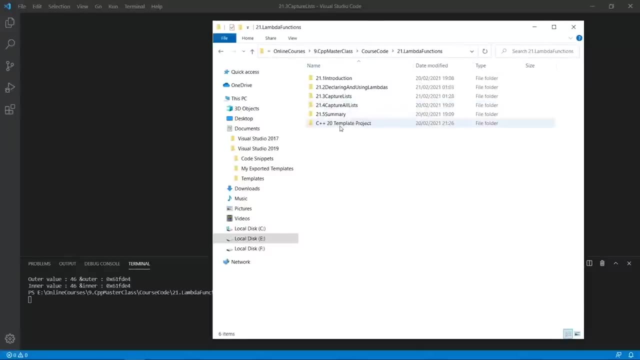 that you know this. we're going to head over to visual studio code and play with us a little more. okay, here we are in our working folder. the current project is capture all lists. we're going to grab our template files pretty quick and we're going to put them in place and we're going to open this little. 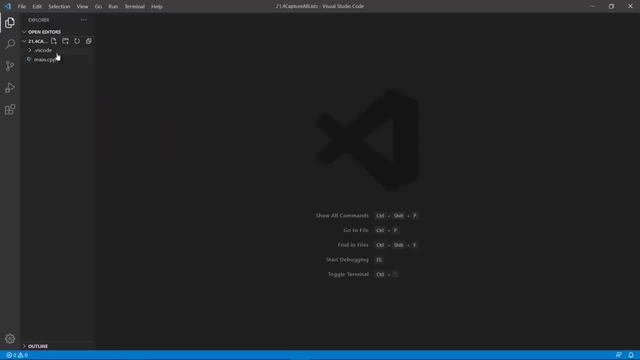 guy in visual studio code. let's do that. we are going to have our folder open. we can open our main cpp file, clean it up, like we always do, and we're going to close the left pane. here, the first thing we want to do is to capture everything by value and we're going to put in the code to do that. 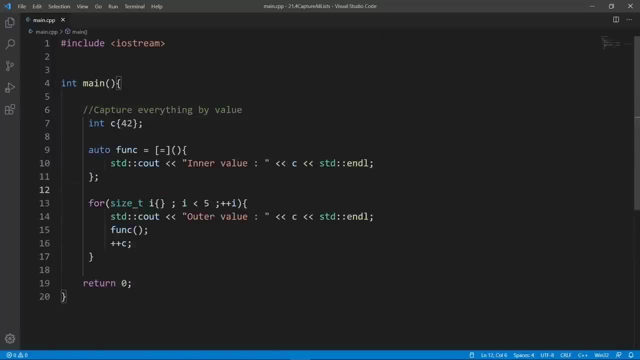 which should be very easy to understand by now and again. the syntax to capture everything by value is by putting an equal sign within your capture list. you have to put that within these angle brackets and that's going to capture everything by value now. now, if we run the program, we're going to see. 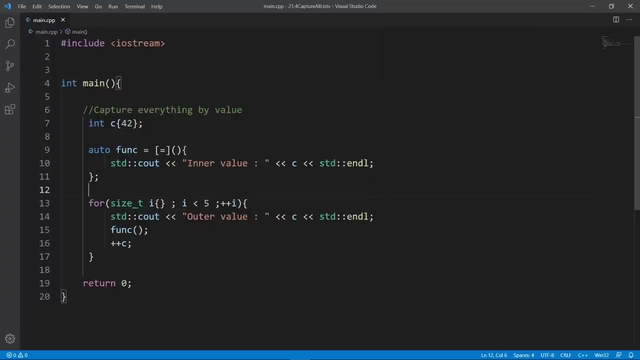 that c has been captured by value. if we look around, we're going to see that the outer value is going to change, but the inner value is going to stay the same. this is the same behavior we have seen before by capturing by value. so let's build again. we're going to build with gcc. the world is. 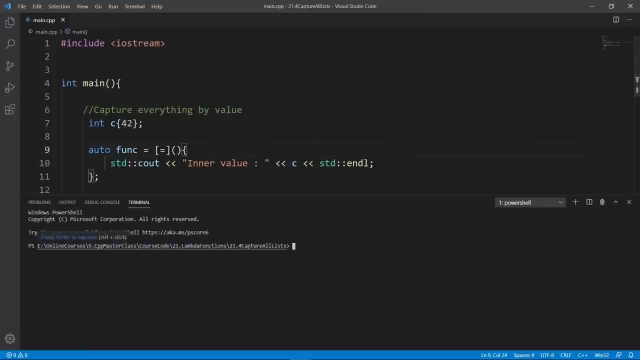 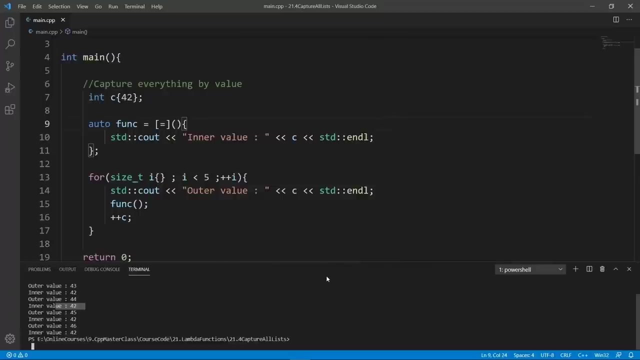 good, we can clear and bring up a terminal so that we can clear properly. so let's do clear and run rooster. now we see that the outer value is changing but the inner value is not changing and again, this is classic capturing by value. if you want to capture all by reference, you're going to 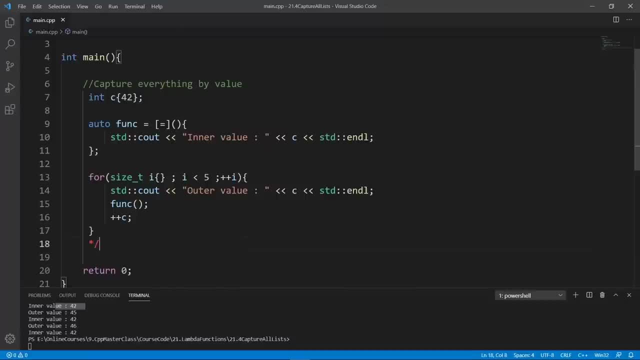 use the ampersand symbol here, and let's do that. we're going to comment this out and we're going to take this out and use the code here. we're going to go down and put in a code and say that we are capturing by reference. we should say: 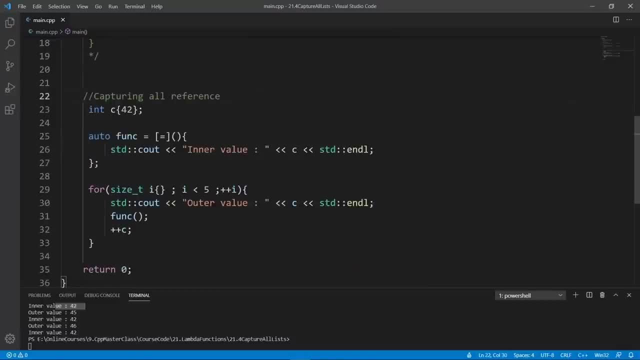 capturing all by reference. and all we have to do to make that work by reference is to put our ampersand symbol within this angle brackets here, and this is going to capture everything by reference. if we run now, we're going to see that the changes we do from the outside are going to be visible. 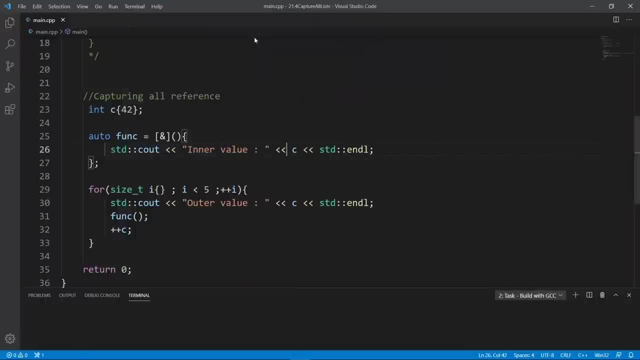 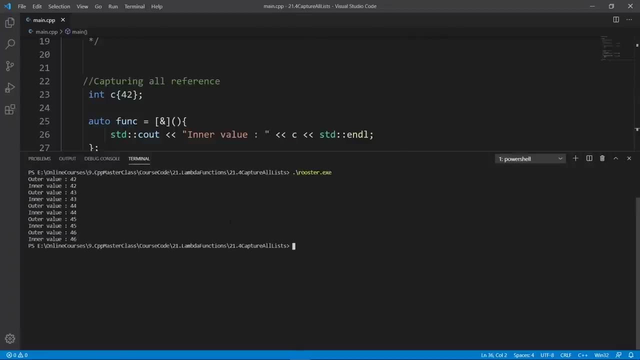 from the inside. here let's build with gcc and see that this is actually the case. the world is good, as you see. here we can clear and run rooster. we're going to see that the outer value is 42. the outer value is changing and the inner value is changing. 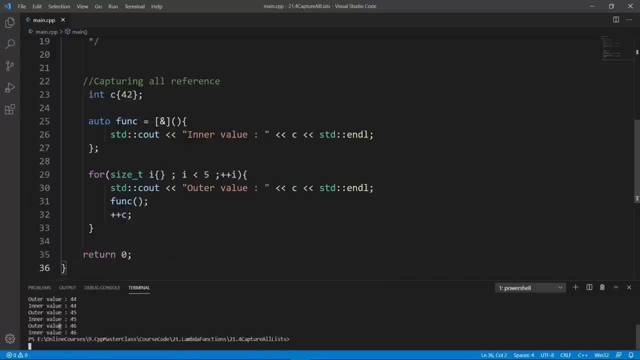 as you see in our output here, and this is really how you can capture by reference. just to play with this, we're going to set up another variable, call it d, and we're going to say it contains a 5 and we can try to print that inside our output and we're going to say that we're going to print that. 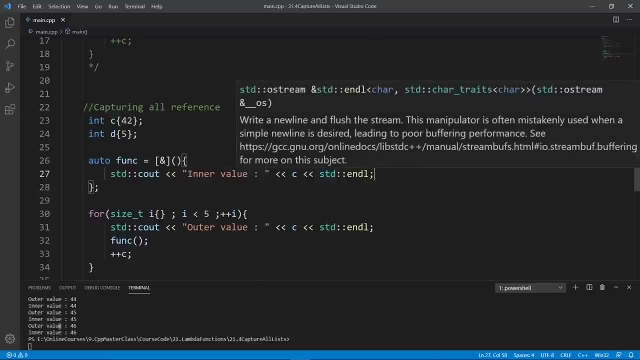 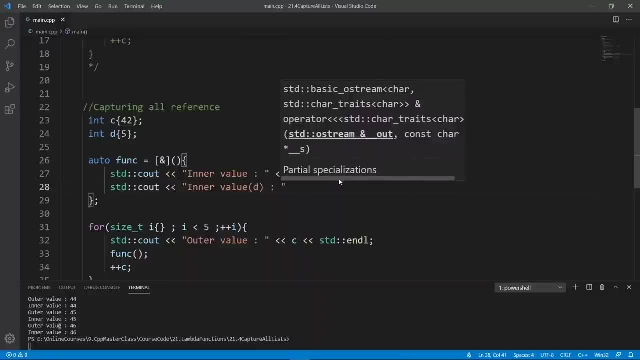 our inner value here and it is going to work. you're going to see that it has been captured. we can say sddc out inner value. let's say that it is the d variable we are trying to access here and we're going to say d and it is going to be visible inside our lambda function here, because 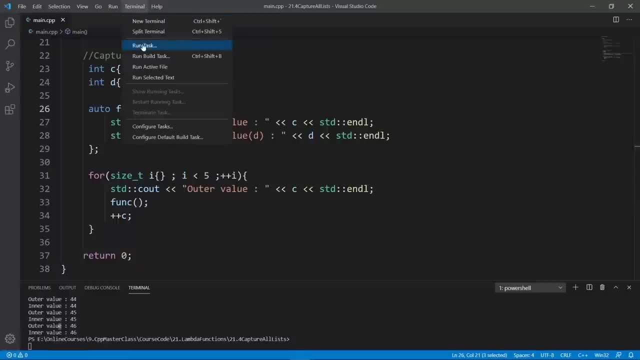 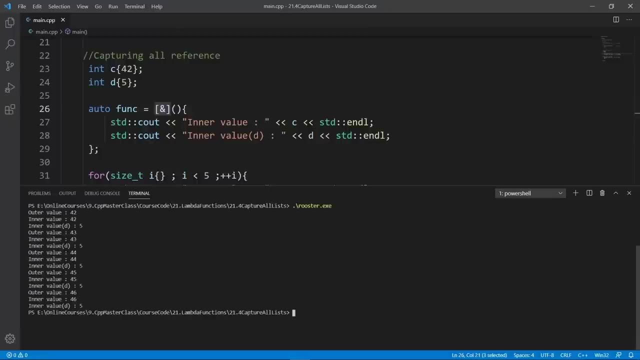 it was captured by reference. here. let's weld again. we're going to use gcc to do that. the world is good, we can clear and if a run booster, we should see d printed out multiple times- d, d, d, d- and we are able to access that through the capture mechanism and we are capturing everything. 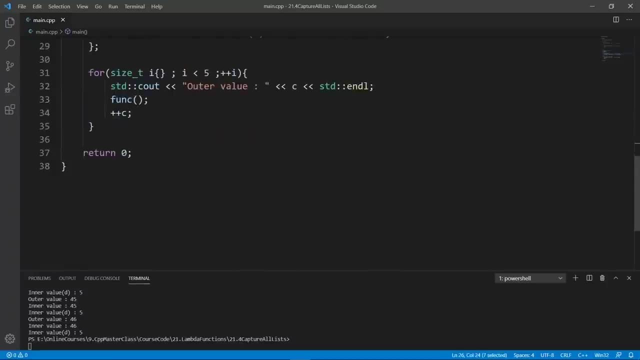 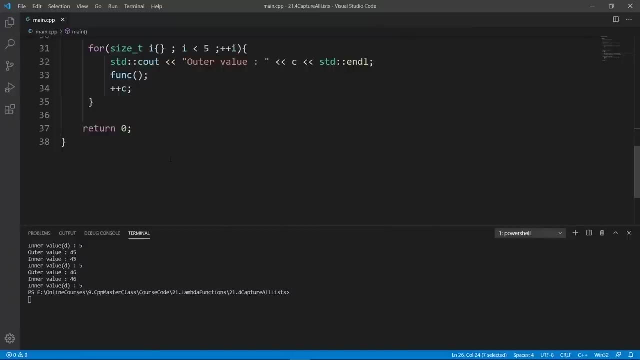 in the context by reference here. this is really all we set out to do in this lecture. i hope you found it interesting. i hate to say it, but this happens to be the last lecture in this chapter on lambda functions. we still have a lot to learn about lambda functions, but unfortunately we don't. 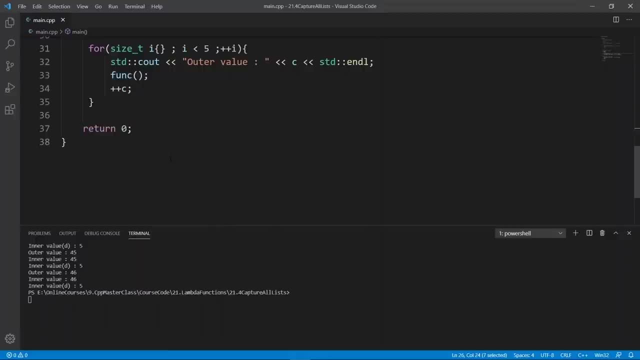 really have enough tools to understand that now. but for now we're going to see how we can do that. we're going to stop here and learn a little more things about c plus plus. then we're going to come back and see some crazy things you can really do with lambda functions. i would like to welcome you. 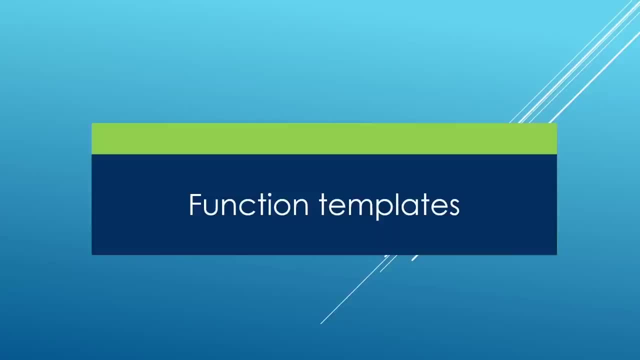 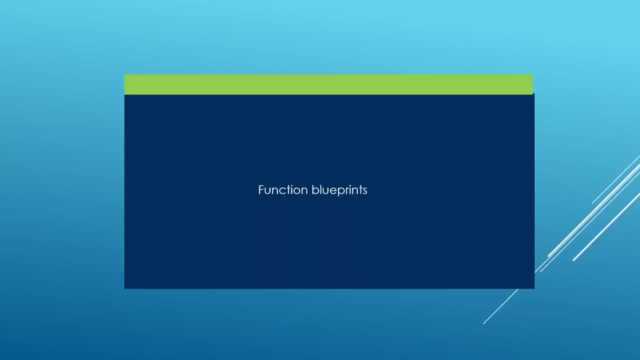 in this new chapter where we're going to be learning about function templates. function templates are a mechanism we have in c plus plus to set up blueprints for functions and have one point of control to set up the function, but the compiler is going to generate the actual function. 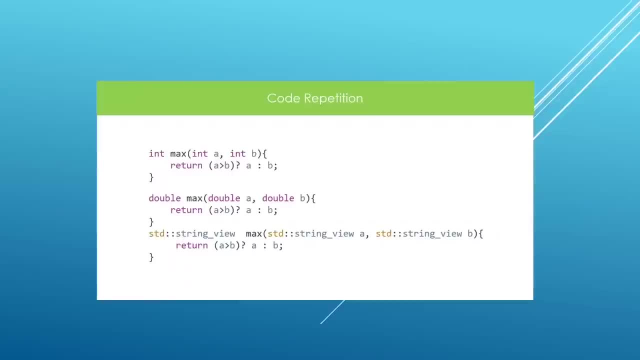 called when it sees the function called. so this is going to solve the problem we had before with function overloads. if you look at the code here, we have multiple overloads for the maximum function, but what we really are doing in the body of these functions is the same, and i suppose you have. 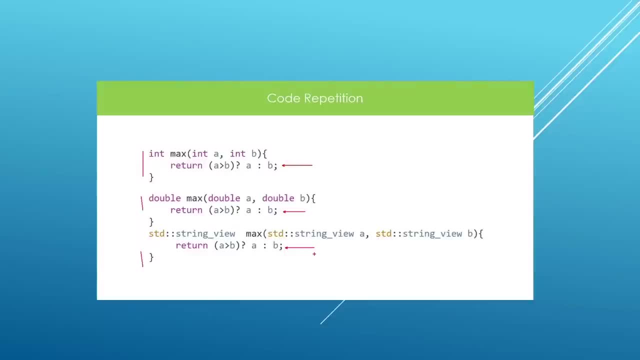 12 or 13 or 20 overloads of the same function. you're going to be basically repeating the same logic in the bodies of this function and this code. repetition is bad. function templates are an effort to solve problems like this. the way they work you set up. 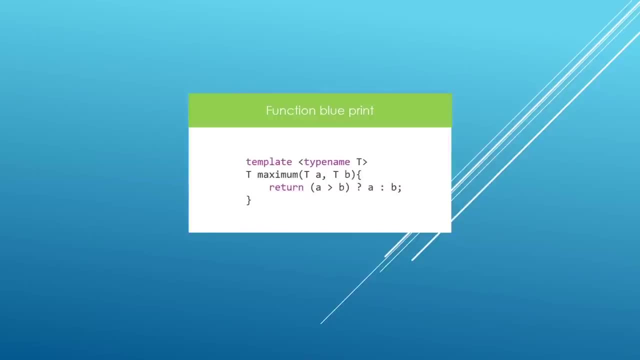 a blueprint for your function and this is the syntax to do something like that. you say template, type name t here. don't worry about this syntax, we're going to have a chance to go through it in detail, but if you do things like this, this is going to be a blueprint for your maximum function. 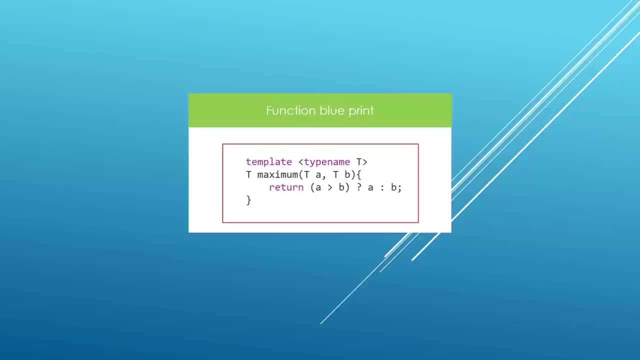 and the compiler is going to use this blueprint to generate an actual function when you call this function, and this is going to make things super easy. i realize some of this is really cryptic, so let's head over to the next lecture and let you set up your very 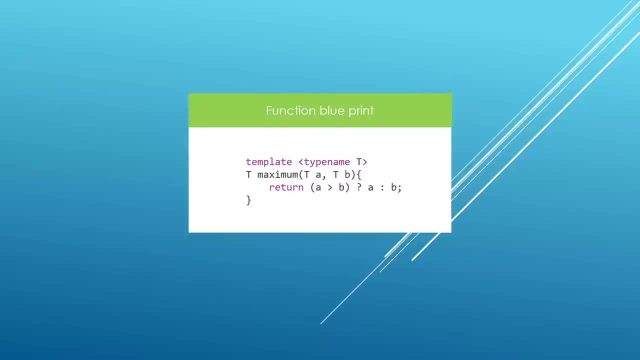 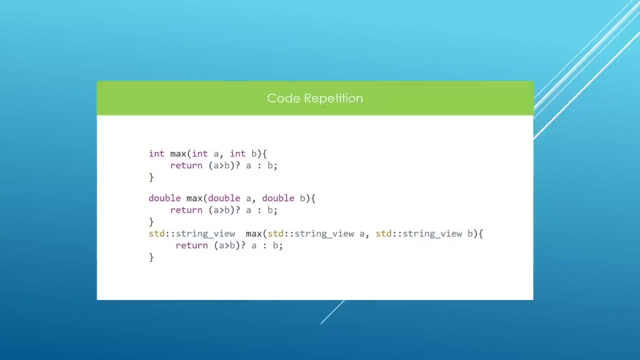 first function template. go ahead and finish up here and meet me there. in this lecture we're going to set up our very first function template. and again, function templates are a mechanism we have in c plus plus to avoid code repetition. for example, if you are setting up a function template, 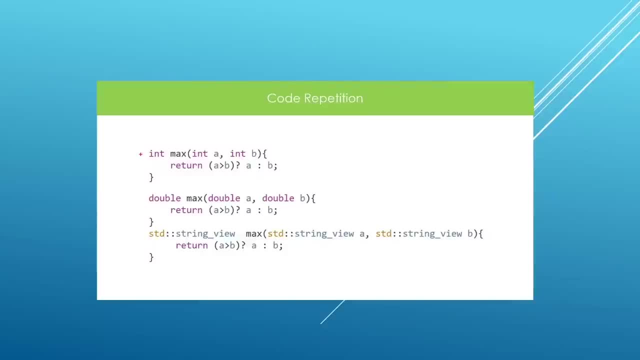 you can use the function template to set up function overloads. if you look here we have our max function and we have multiple overloads for this function. we can call it with ant double and string view here. but if you look inside you see that we really are repeating the same logic. 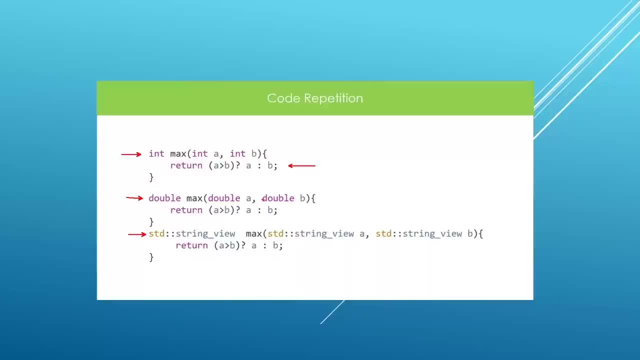 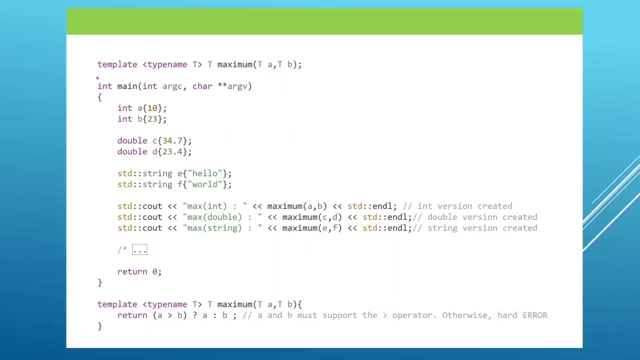 and it is even possible to have dozens of overloads if you want to support tons of types for your function and this code repetition is really bad. so we're going to set up our very first function template and we're going to set up a function blueprint using the syntax you see here, and your function template is going to be prefixed. 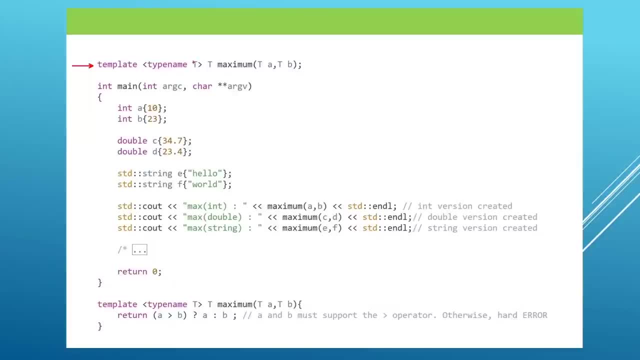 with this template type name t thing here type name t is going to be in this angle brackets and then you're going to put the blueprint for your function. t is a placeholder for the types that you use in your function. you see that t is a placeholder for the types that you use in your 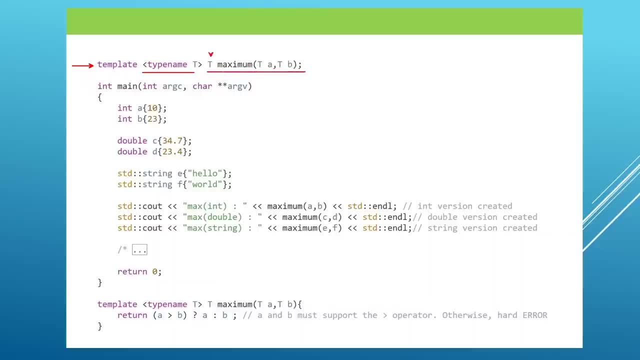 function. you see that t is in the return type here. it's in the parameters that we pass to the function. and because it is the same character here, all these things have to be of the same type: the return type, the first parameter, the second parameter. they have to be of the same type, okay. 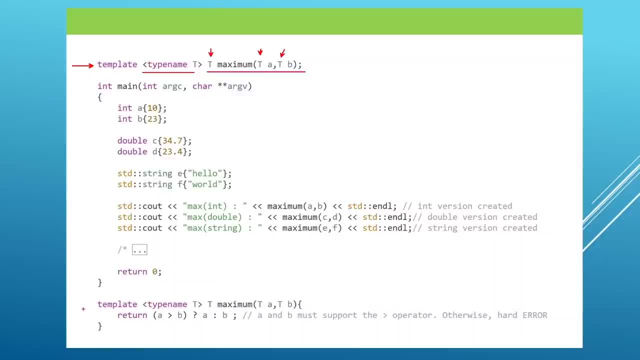 so once you have your function template set up like this, you're going to implement it like we see down below here. it is nothing complicated. we just set up the prototype for the function. on top we put our implementation. you see here we have separated this into function declaration and 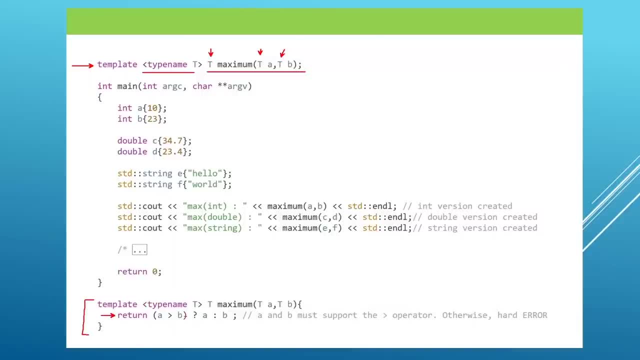 function definition. but inside you see that it is the same logic. we had to compute our maximum between these two parameters that we pass to this function. so how does this work? when the compiler sees you call this max function, for example, as we are doing here, it's going to look at the types. 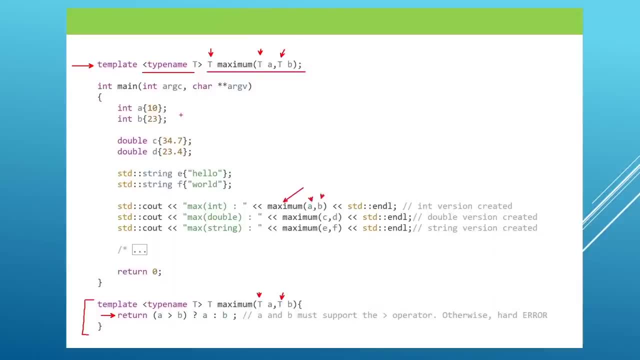 that you pass in, and in this case a and b are of int type, so it is going to replace the t in here for int and it is going to generate a function in your code. and this really brings up a big point about function templates. many people think that function templates are actual c++ code. they're not. 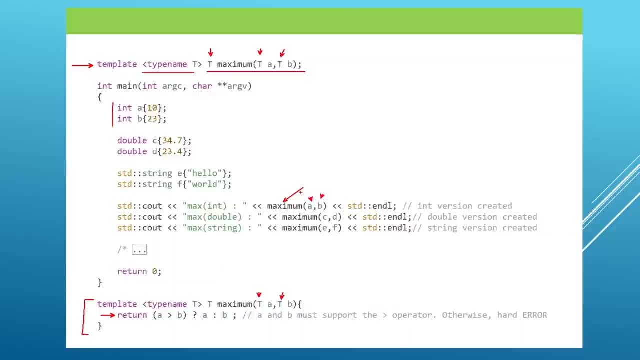 they're just a blueprint from which the compiler is going to generate the actual function that is called by the compiler. and it's going to generate the actual function that is called by the compiler, for example, when you issue a call like this. again, function templates are not real c++ code. 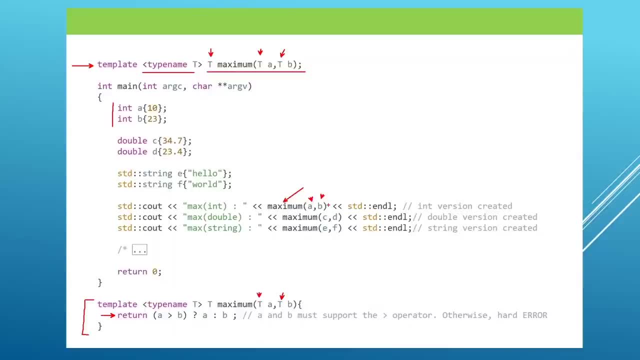 they are just a blueprint that the compiler uses to generate your function based on the arguments you pass to the function when you call it. so when we issue the call, like we do here, an int version of our maximum function is going to be created. so the compiler is basically going to go in and 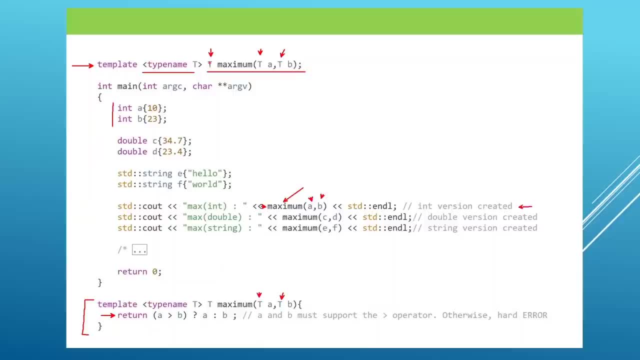 replace n and for t here. the return type is going to be n and for t is going to be n and for t is going to be n, and the first parameter is going to be n. the second parameter is going to be n. it's going to go in the definition. it's going to do that and we're going to have an int function if. 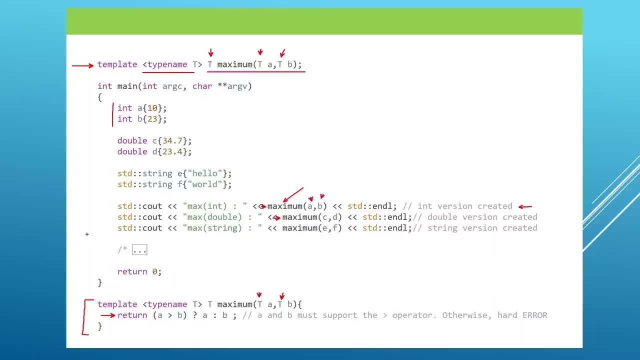 we issue a call with c and d, like we do here in the second line here, then the compiler is going to see that c and d are of double type. so it is going to generate another function from this blueprint here and it is going to replace in double. then we're going to have another double. 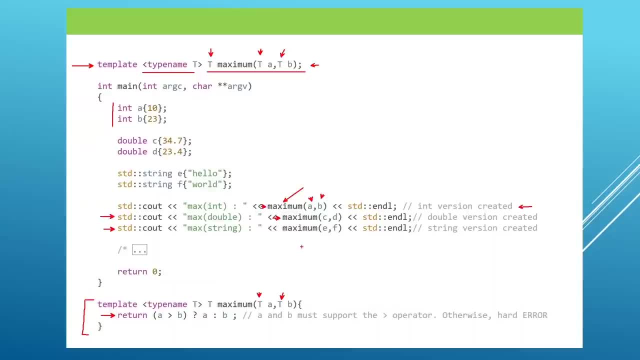 function. if we go to the third line here, we're going to do the same, we're going to call it with, and it is going to generate a string version of the maximum function here. so what we achieve with function templates is to avoid several overloads for the same function and we have one point of. 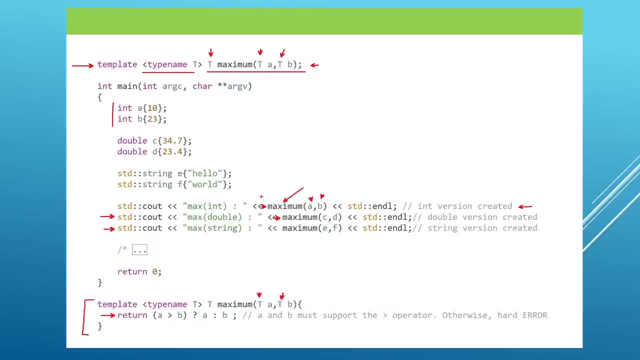 control in our code, but the compiler is still going to generate this function overloads. but one thing about this is that if a function is not used, for example, if you never call a maximum function with string, then the string version is never going to be created. the compiler is going to generate the overloads that you only call in your c++ program and this 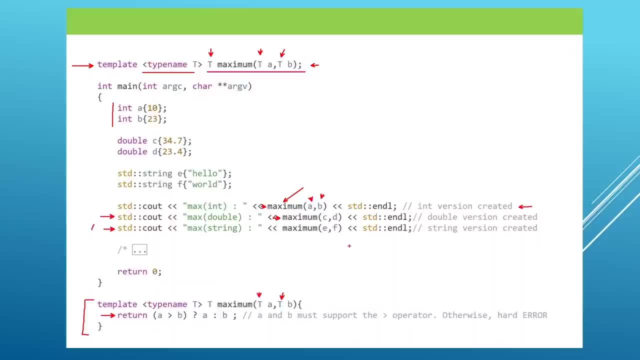 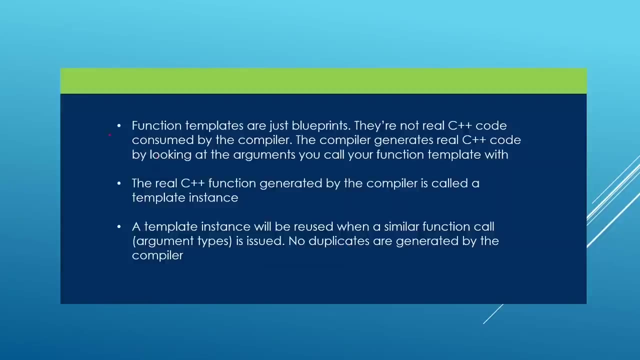 is really all function templates are all about. they give you a mechanism to set up a blueprint for your function and then the compiler is going to generate actual functions based on what you call in your c++ code. okay, we have said this, but i want to emphasize this again: function templates. 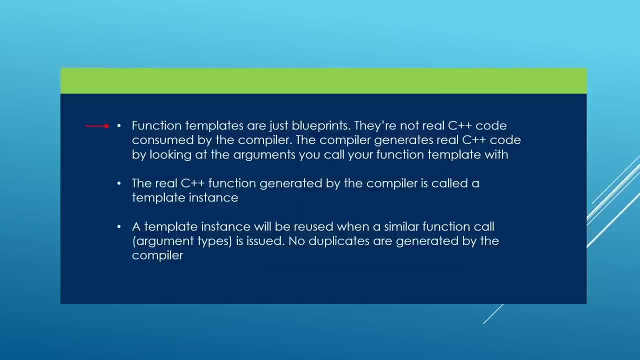 are just blueprints. they are not real c++ code and we hit visual studio code. in a minute we're going to see a tool that allows us to see how the compiler instantiates your function templates based on the arguments you call your function with. but keep this in mind: function templates are not real c++ code. the real c++ functions get generated. 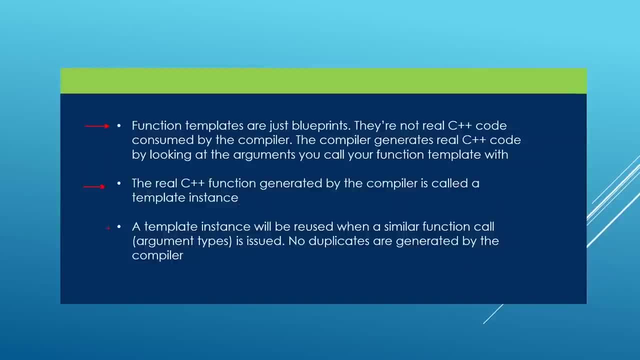 by the compiler when you call your function. and another thing i wanted to point out is that once a function template is generated, for example the introversion of our maximum function template, then if it is needed again, the compiler is not going to generate that again. it's going to see if there is one generator. 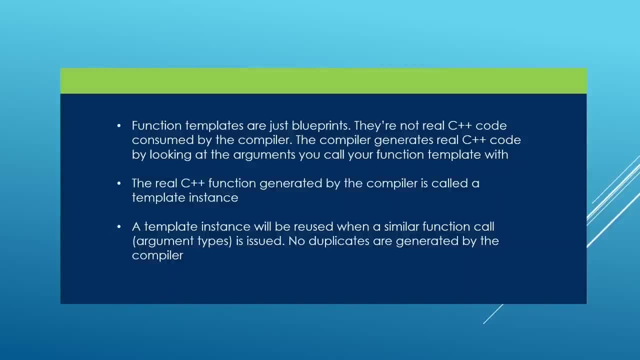 already and it is going to reuse that. okay, this is really all i have to share about function templates at this point in this chapter. for now, we're going to head over to visual studio code and play with this a little more. okay, here we are in our working directory. the current project is trying out function. 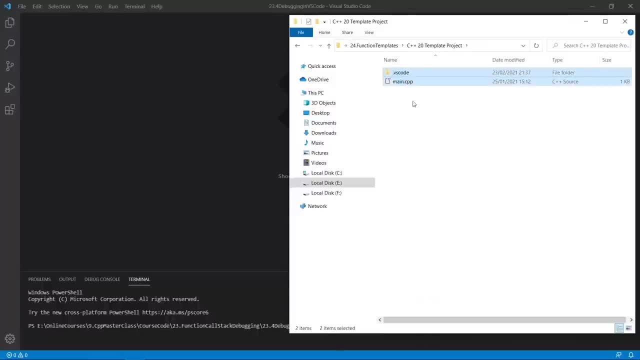 templates. so we're going to grab our template project, and one thing i should point out here is that our template project has been now updated to have the launchjson file, which is going to allow us to debug our programs, so you should use a template that includes the launchjson file here. 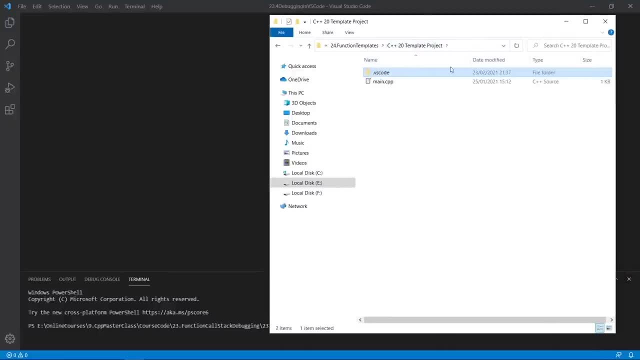 that's going to allow us to debug your programs, and we're going to do that in a minute when we have set up the example here. so we're going to grab our template files and put them in place and we're to open this little guy in visual studio code by dragging and dropping on top here. this is going to. 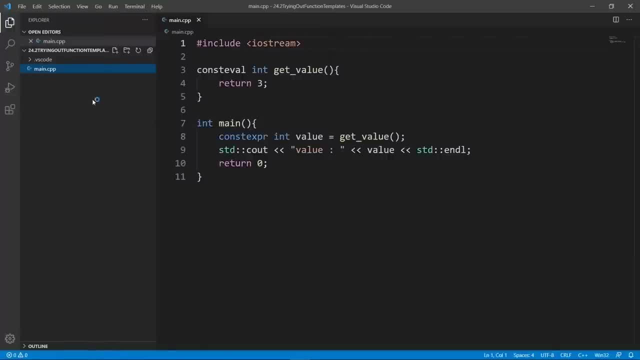 do our job, then we're going to open up the main cpp file and i think we should close the left pane here. we don't need it anymore and we're going to clean this up a little bit. so one thing i want to do is to first do things the bad way. so we're going to set up a max function. let's call this: 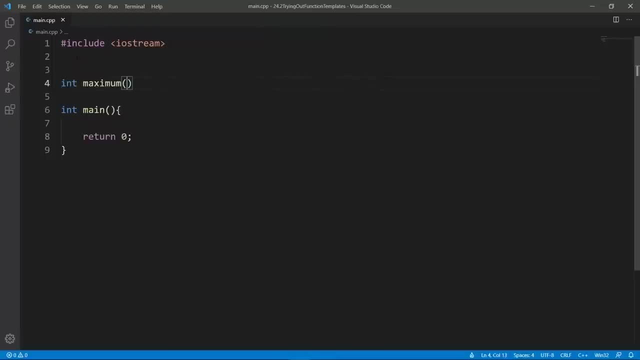 maximum and it's going to take int parameters and we're going to return the maximum between a and b and the way we do that, we say a greater than b. we are going to use our ternary operator here, we're going to put a question mark, we're going to return a or b and this is going to be our function. but 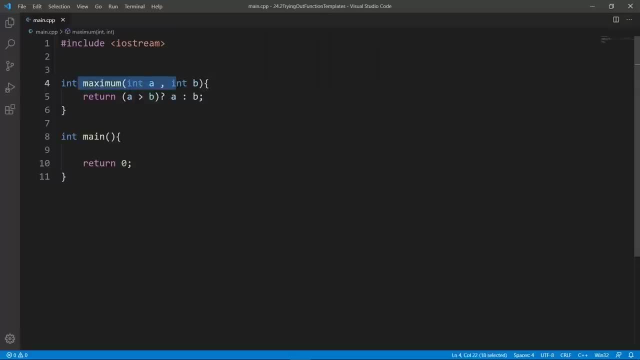 suppose we need another function that works on doubles. if we put double arguments in here, the compiler is going to insert implicit conversions from double to end. this may seem to work, but suppose you use a parameter type that is not convertible to end, for example, you use a string. 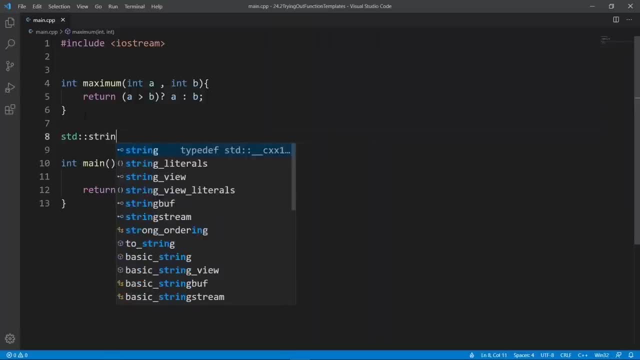 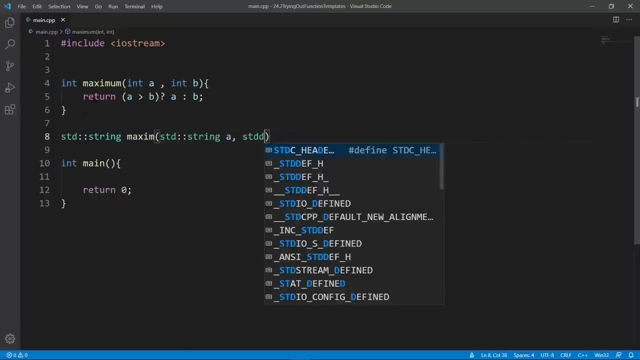 or something like that, and you use a parameter type that is not convertible. to end, for example, let's put in std string here, just for an example. so we're going to say maximum std string a and std string b, and we should make this const references, because we're not interested in modifying these. 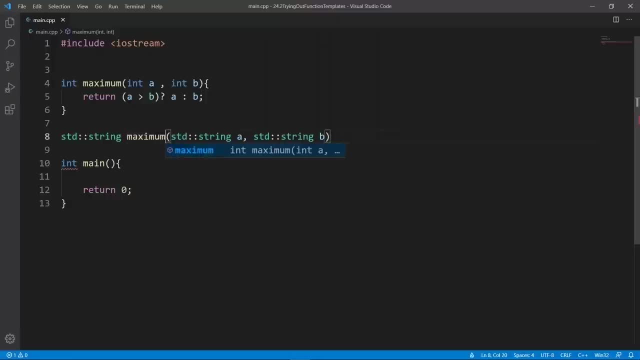 strings here. let's finish the name here and we're going to say const std, string reference a. this is much better. it's going to avoid unnecessary copies of strings. and we're going to say const std, string reference b here. then inside, we're not going to do anything different, we're. 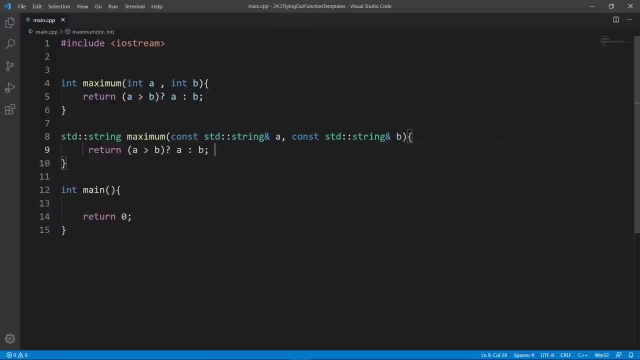 just going to use the same logic. okay, let's do that. suppose you have another function which takes what should i say long, long, and if we need that, we need to copy this function and put that in. okay, we need to do that, and we're going to change this to long, long, and, and we're going to do the same. 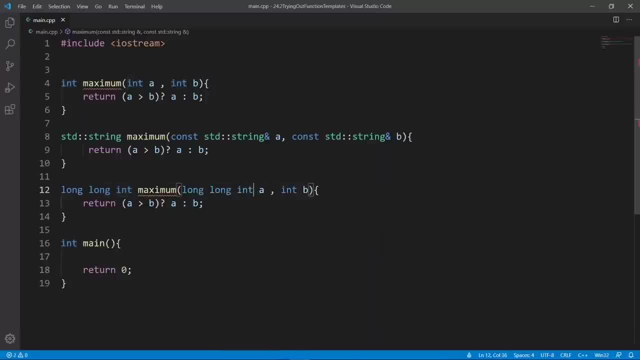 here long, long and our and we're going to say the same here, and you see we are setting up a lot of functions with basically the same thing inside and that this is a lot of code copies. suppose we have this function: maybe 20 times it is possible, or even worse. the logic in this function is really long, maybe 20 or 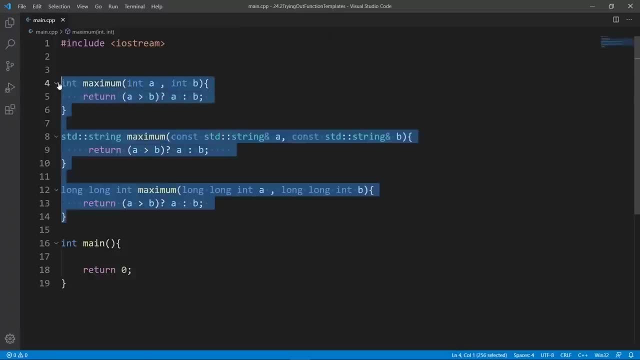 30 lines and we will have to repeat this thing in our code. so the designers of the c++ language saw this problem and they said: why don't we do this? and we're going to do this, and we're going to do this? we set up a one point of control where we can set up our logic to do the maximum and we let the 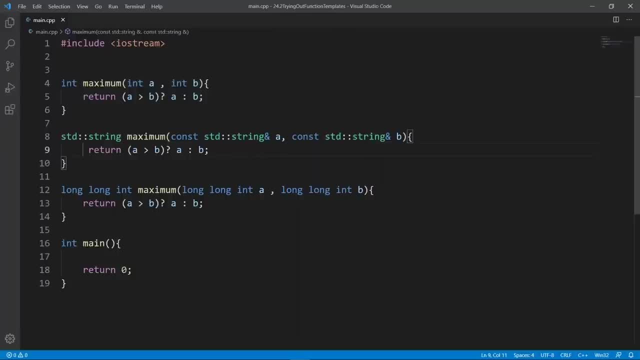 compiler generate actual functions based on the arguments we call our functions with, and they came up with function templates, and that's what we're going to see. so we're going to take out all the other functions and we're going to turn this maximum and function into a function template. 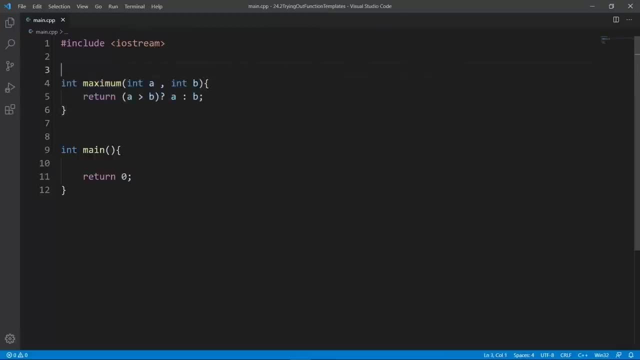 the syntax to do that is ridiculously easy. we're going to say template- this is what you say. you put an angle bracket and you say type name and you specify the placeholder for the type in this angle brackets here. this is the syntax you have to use. then you have to specify your function in terms of this placeholder t. it is going to take. 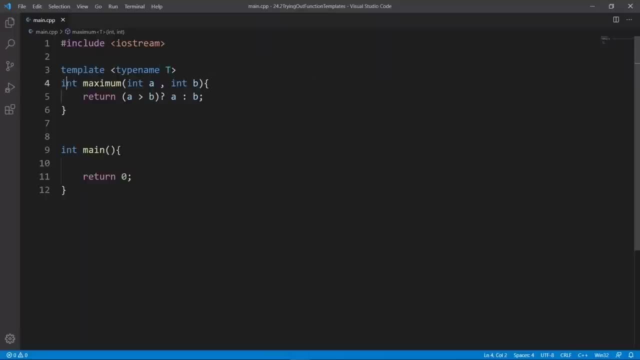 the place of the type. so, for example, here we want to return and we're going to change this to t, and the parameters are going to be taken by value t and t. this is how we're going to set this up, whichever way is working, because what we're getting on now? 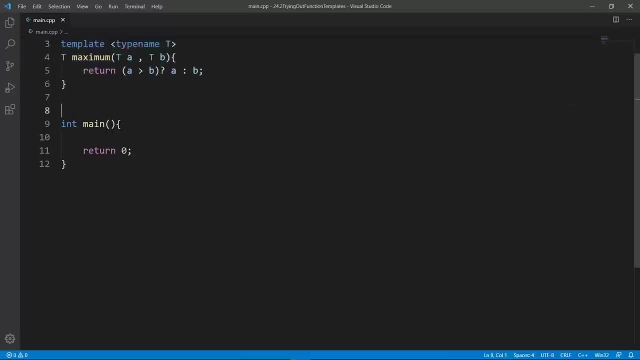 is, we're going to be an echo, so we're going to gather in these variables we should have, should be Tran and we should, and, and this is going to be t and t, t and so, for example, we, when we're leh shows, we move those to the. here is sort of the state of c plus plus, and then there is this: 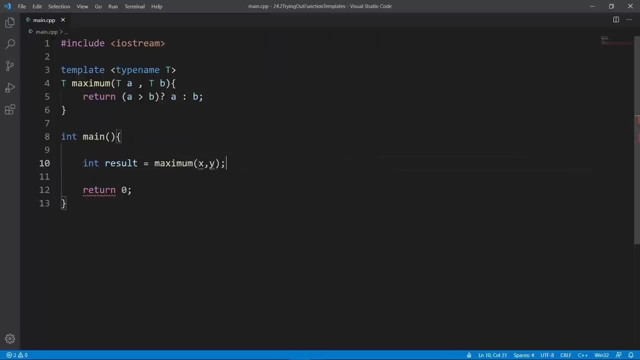 element which shows x and y. so if we move this out we should see x and y is actually aY, not fy, and that's what we want to have on the, the table, the table center in the, on the table center of the table centersir. 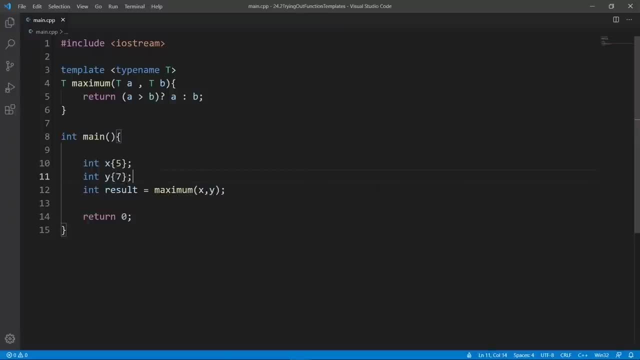 put and a 7. why not now? this function is going to store the result and print it out. let's do that so that we can see that this actually works. so we're going to say result and say result. this is going to do, and if we build and run this program, we're going to use gcc. you're going to see that. 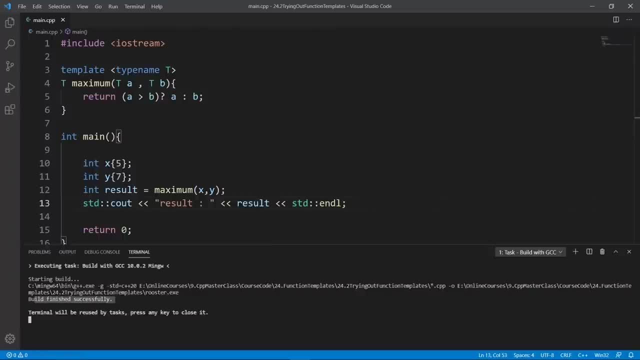 the world is going to be good and, uh, well, finished successfully. we can run this program like we always do. let's bring up a terminal and clear a little bit and run roaster. you're going to see that. we're going to see that result now is 7, because that's the maximum. you see, it is working. 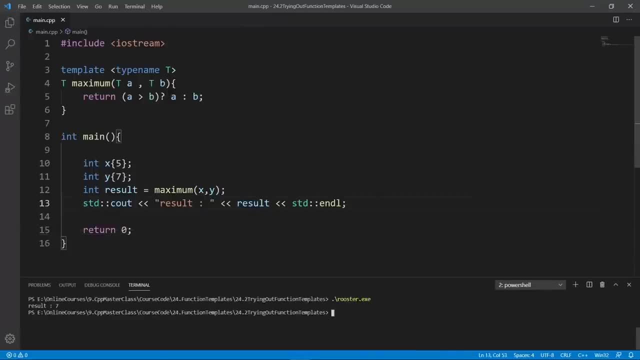 here. so how is this mechanism working here? the compiler is basically looking in the main function here and it is noticing the call and it is going to look around and see if it can find a declaration for the maximum function here. it's not going to find it because there is none. 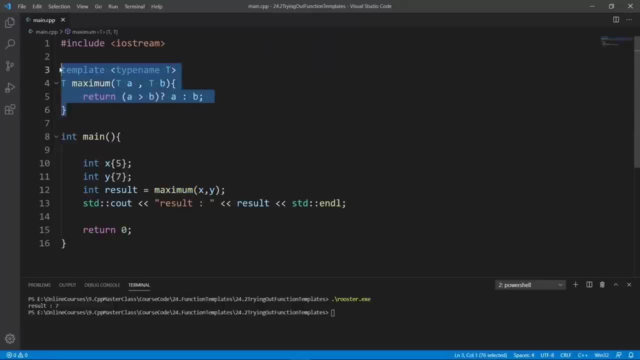 then it's going to look around and see if it can find a declaration for the maximum function here. so it's going to look at the function templates it has in here and it's going to see that it can do a replacement and replacing the types that we are passing in here. so it is going to do that. it. 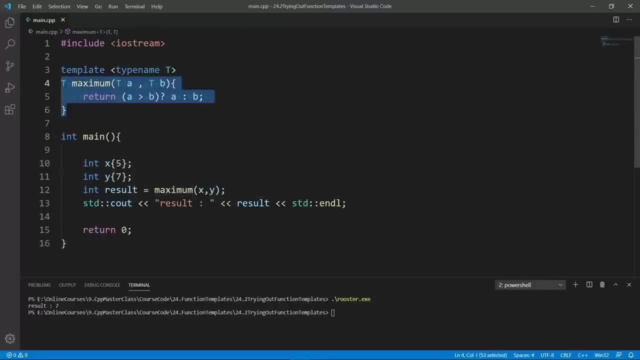 is going to take this template and it is going to replace t by end, and then it is going to generate a function that basically looks like what we have here. we're going to copy this and we're going to put this in. the compiler is going to take the first t here. it's going to turn that into a net. 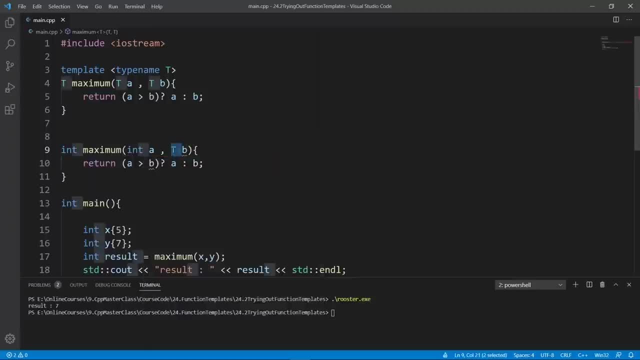 it's going to take the second one here. it's going to turn that into a net, it's going to take the third one here and turn that into an int, and we're going to have a function definition for the call here. this is what the compiler is going to do. one thing some of you might be thinking: is there a? 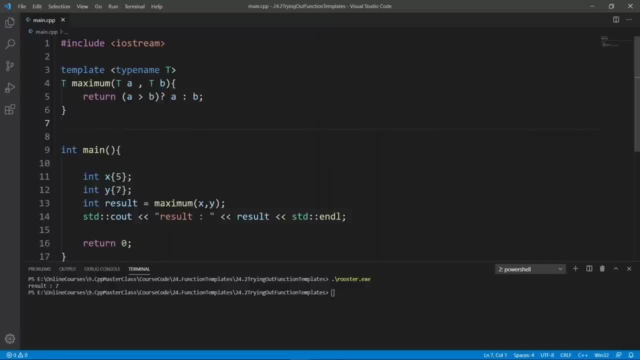 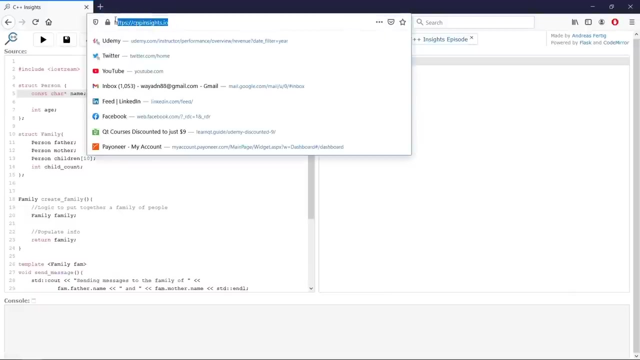 way to really prove this, and somebody was nice enough to design a tool to let us see this function or template instances generated by the compiler, and I happen to have that opened. it is a web-based tool, so you can use this in your browser. just go to cppinsightsio. 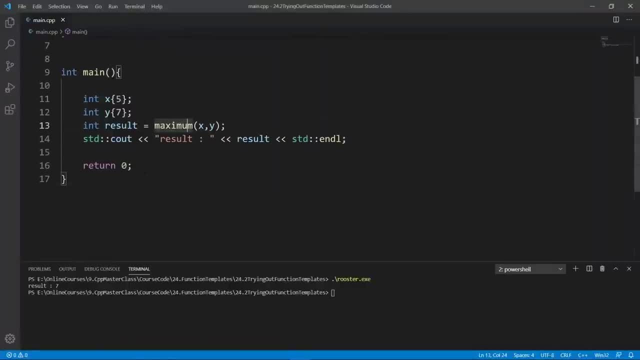 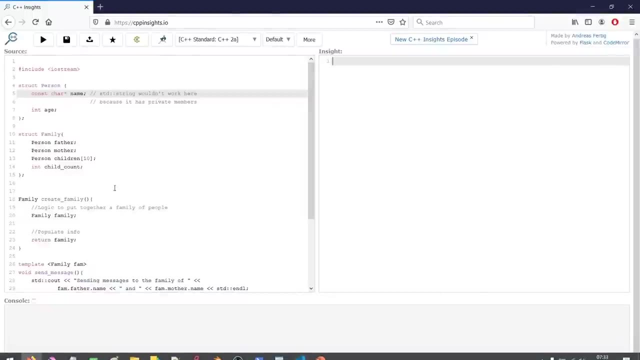 and then we're going to grab the code we had in our main cpp file, we're going to copy it all and we're going to go back to our browser and remove whatever I had in here, because I don't want this anymore, and I'm going to put in my function template. if we want, we can even take this. 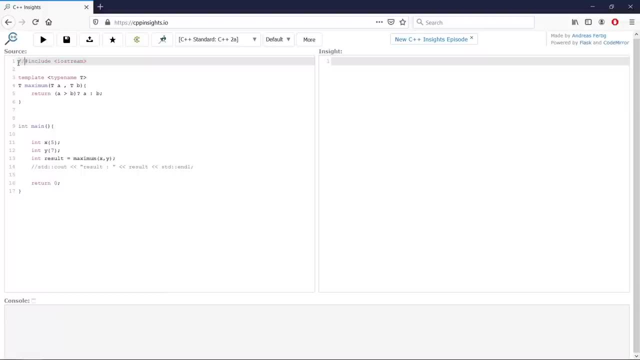 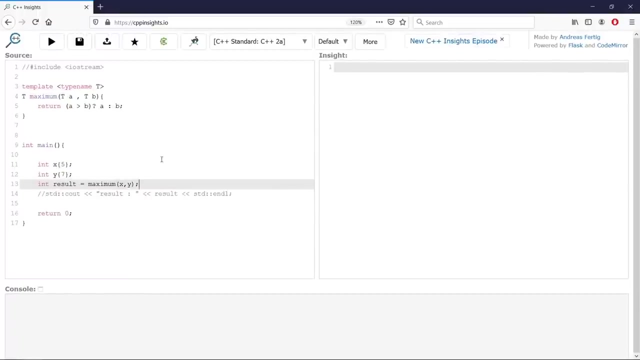 link that comes with that. we are just interested in looking at the template instances generated by the compiler. now that we have the code in here, we're going to see what the compiler generates because of the call we have here. I think I could increase the size of the font here so that you. 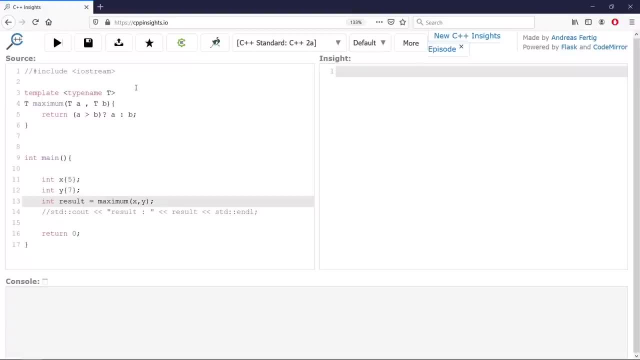 guys can see this. I think this is a little better then. if you head to this play button here, let's click on it. it's going to do its processing and then the code generated by the compiler is going to show up to the right here. you see, it has detected that we have called. 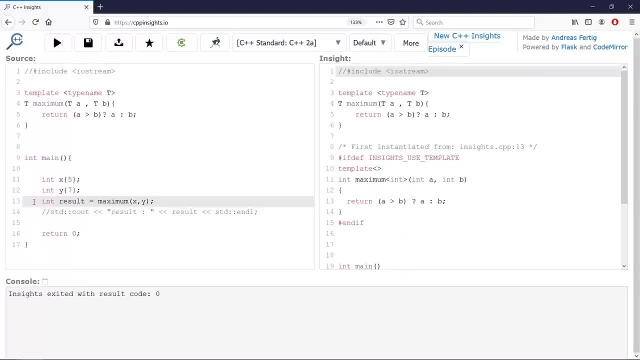 the function template on line 13. here you see this line is highlighted and then if you go to the right, we're going to see the functions generated by the compiler. so if you go here, you see that we have an interversion of our function template. and another thing I should 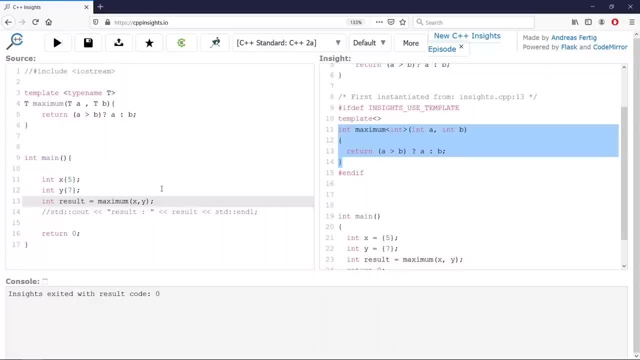 prove here is that template instances that are not needed are not going to be generated by the compiler. anyway, to save us, the compiler is only going to generate the template instances it needs, and again, a template instance is what you have here, the function, the actual function that is callable. 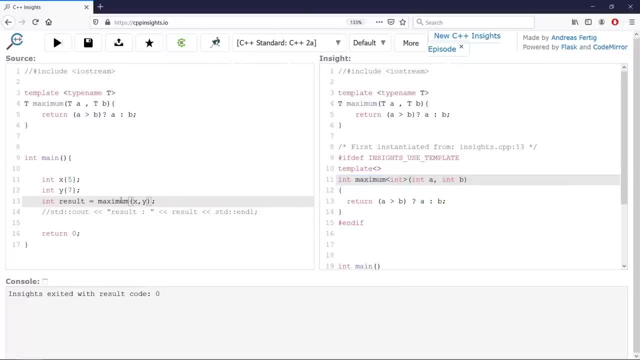 by the compiler, generated from your blueprint. so if, for example, we change the type of our parameters to double, let's do that. okay, so we changed our types to double. we're going to hit the play button again. you're going to see that now it is going to generate. 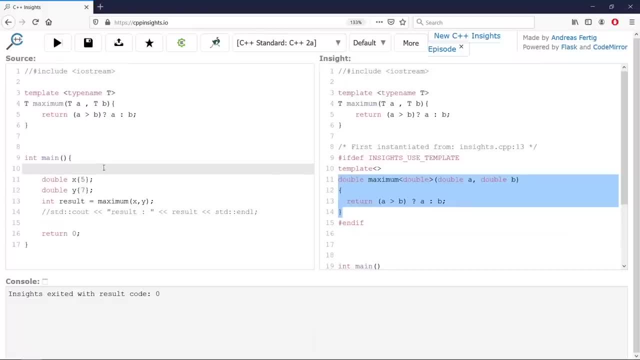 a double function here. you see that here, if we change this, for example, to what can we use? let's use long, long end, like we did in our lecture. we can do that. we can say long, long end and if we hit the play button, that's what is going to be generated by the compiler. so hopefully this proves. 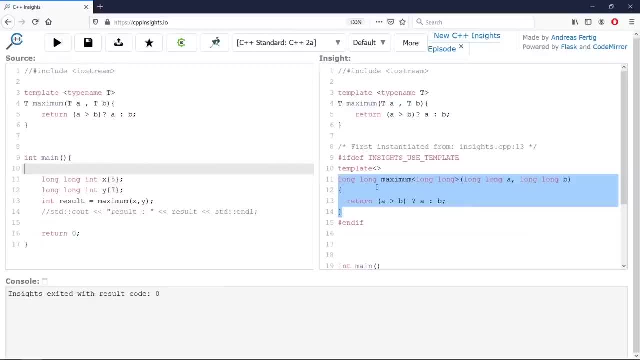 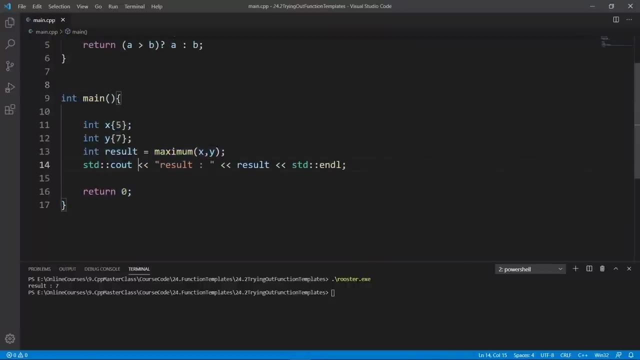 that the compiler is only going to generate the instances that are needed for the calls you do in the program, and this is really function templates are all about. okay, now that you know this, let's set up a few more examples to see that this really works. so let's change the types of this, guys to. 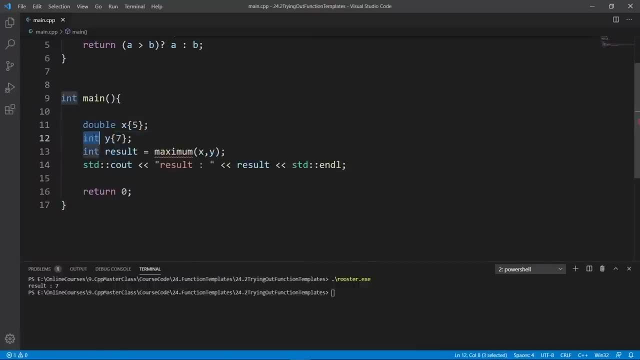 double. let's do that, and we're going to play with this a little more in the Visual Studio code. and let's use double literals, 5.5 and 7 or 78.7 here. let's do that- 78.7, and we're going to build this. 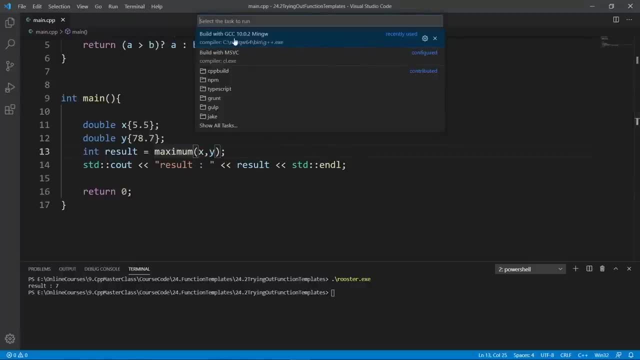 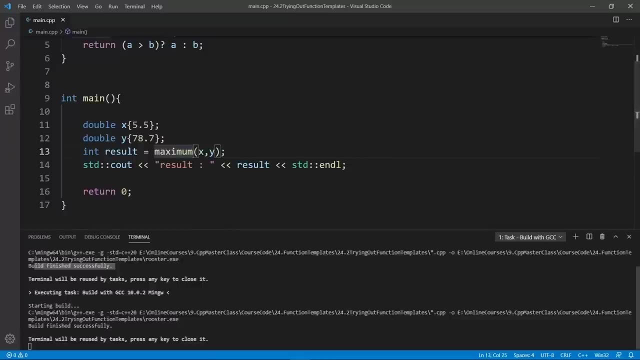 and one thing I should point out is that template instances are generated when the compiler is doing its job, and then they are going to be put in the binary representation of your source code. so the world is good. as you see, here we can clear and run a roaster. we're going to see that the result is 78. 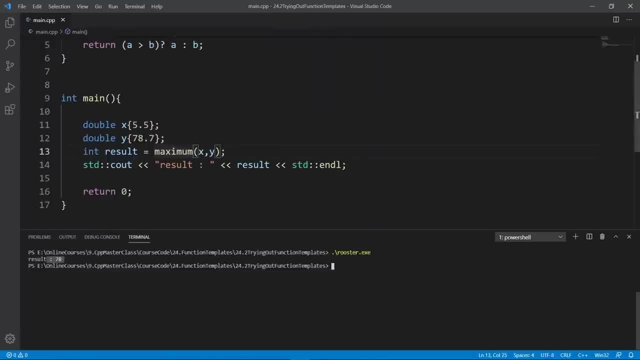 and it is transformed to end, because we are assigning to end here. to really get the correct results here we should use auto type deduction. if we do that, the compiler is going to deduce the type of result here based on the return type of this function or the function template instance. I should say now we're going to change this to: 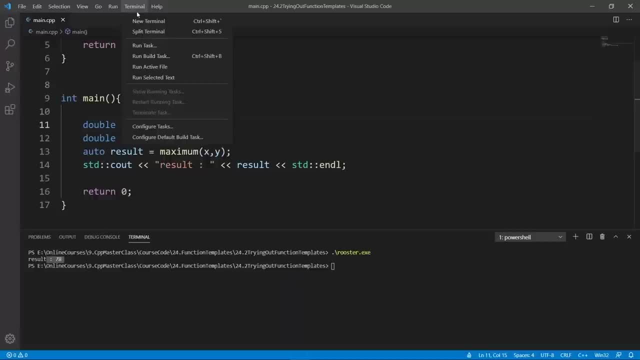 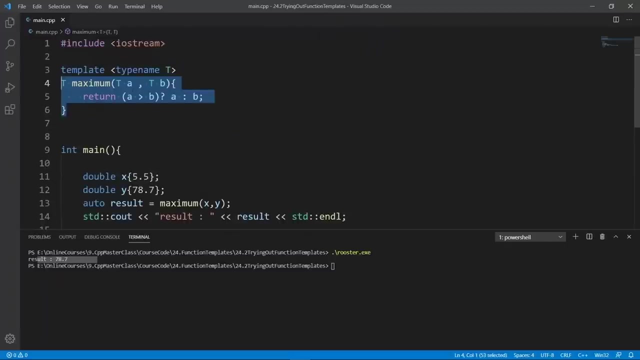 auto to do auto type deduction. and if we both again we should see a double printed out correctly. the world is good. we can clear and run roaster. now we have the correct value printed out from our function template here. let's change this to std string. we can do that. 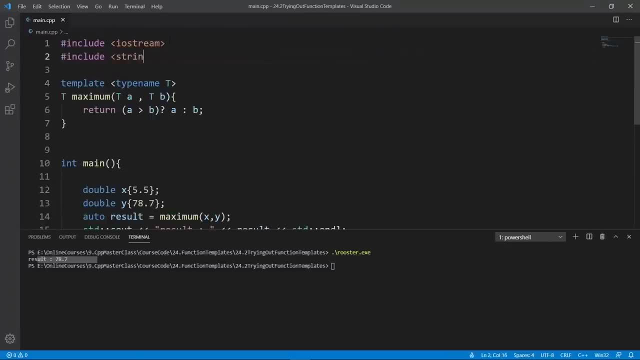 so let's include a, the string library, and we're going to change these two guys to std string. why not std string? x is going to be a string, literal. let's use hello, for example, and uh for Y. we're going to say std strength and we're going to put in a world here. okay, this is going to do, and you. 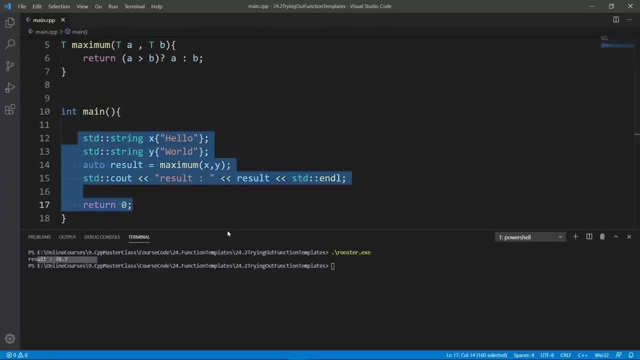 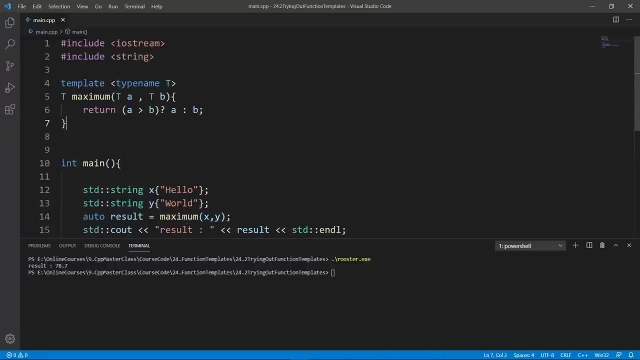 notice that we don't even have a compiler error. Visual Studio code is not complaining. the compiler is going to look at the types we call our function with. then it is going to generate a nested string version of this function and what it is going to do. it's going to replace in T and replace that for. 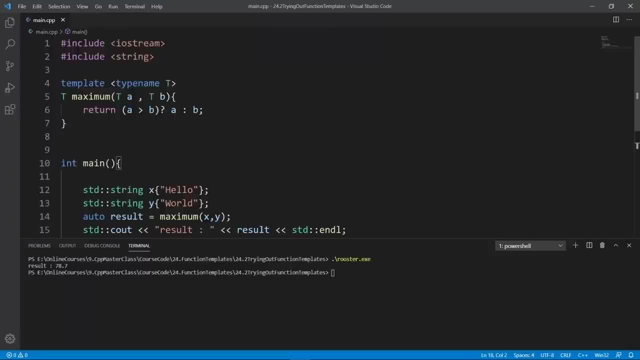 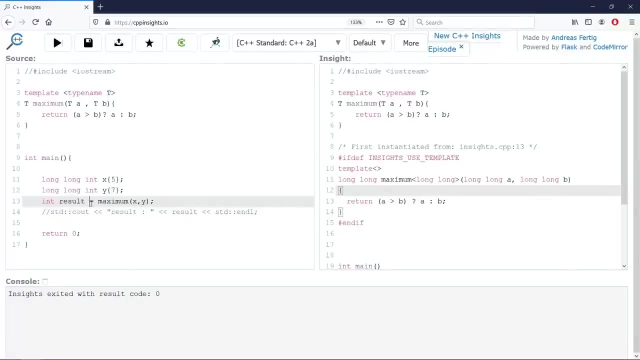 std strength. we can actually put this thing entirely in uh cpp inside. so let's copy this code before we run it, so that you can really see what is happening here. we're going to take out whatever we had before, we're going to put in our code and then we're going to hit the play button. here it's. 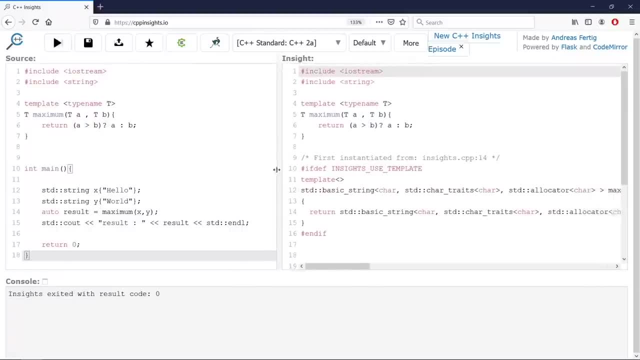 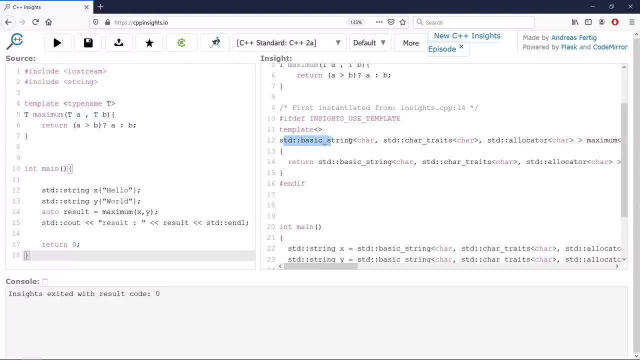 going to generate our thing. we wait for it to do its thing and if you look here, you see that it has generated std strength. this is really a compiler representation of std string. we don't have enough tools to really understand this, but hopefully you can see that it has replaced T with some other type. 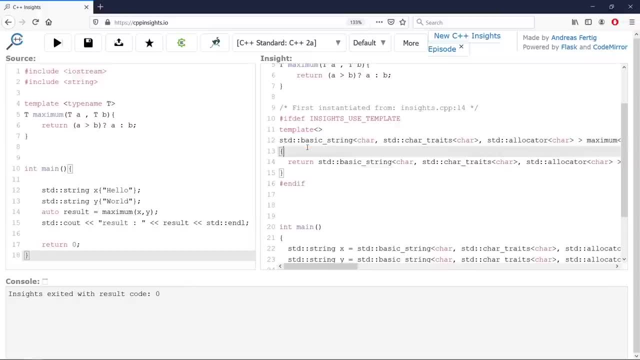 we don't know yet. std basic string car. it has a few things inside that we don't really know yet. we will have to learn a few more things about this as we progress in the course, but for now I want to prove to you that the compiler is. 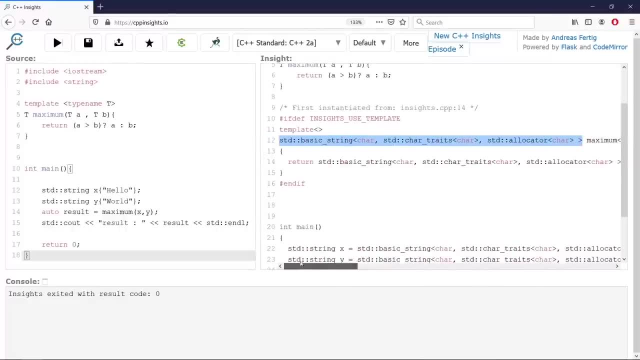 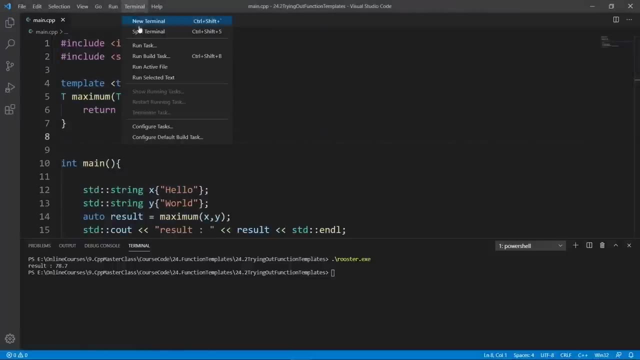 doing the replacement. you see, T was replaced by this thing here- std basic string, and we have angle brackets and this entire thing is really std strength in the eyes of the compiler. okay, now that we know this, let's go back to Visual Studio code and run this. we're going to build with gcc. 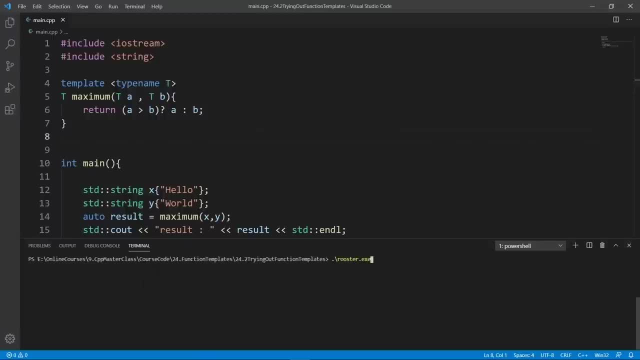 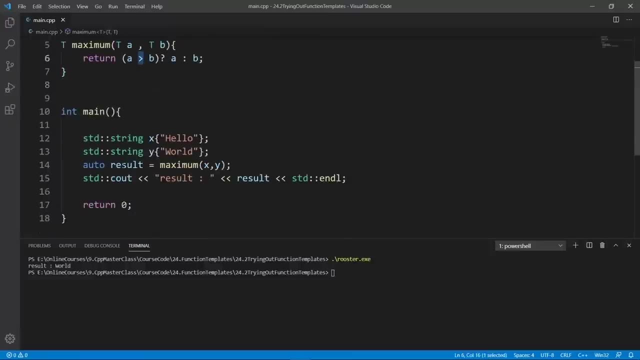 as we always do. the build is good, we can clear and run, rooster that the maximum is world and this is going to be using the greater than operator and this is going to compare two strengths. based on this- and we know that W here comes after H in lexicographical order- 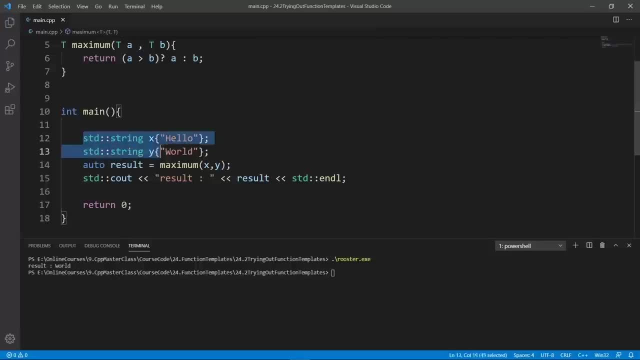 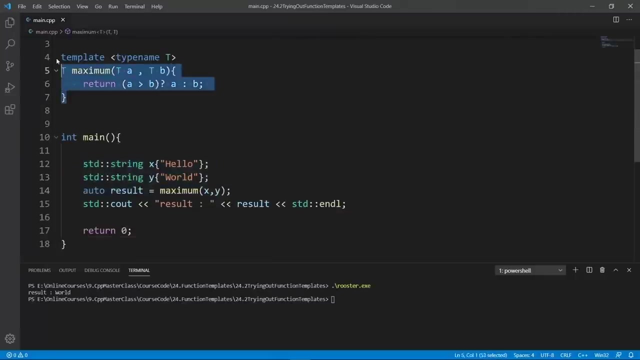 so the comparison that is done here is lexicographical for this strength here, or I should say it is comparing things in alphabetical order in a, b, c, d, e and things like that. okay, now hopefully you have a big idea about function templates. they are just blueprints you use to generate actual functions and this is going to 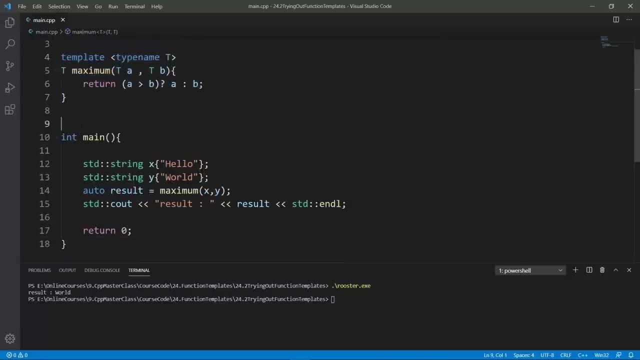 allow you to avoid multiple function overloads, as we have seen before. one thing I want you to see is that you have to be sure that the logic you do inside your function is supported by the types that you pass to the function, and I'm going to show you what I mean here. we're going to set 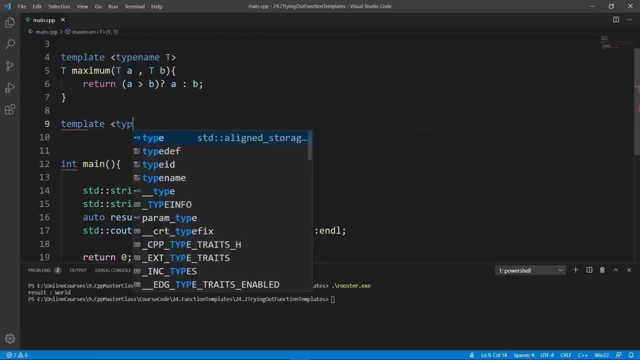 up another function- template. we're going to say template, type named. we're going to set up another one and we're going to use T here. you can use this however many times you want. and then we're going to set up a function which is: you're going to do a multiplication, so we're going to say T, that's. 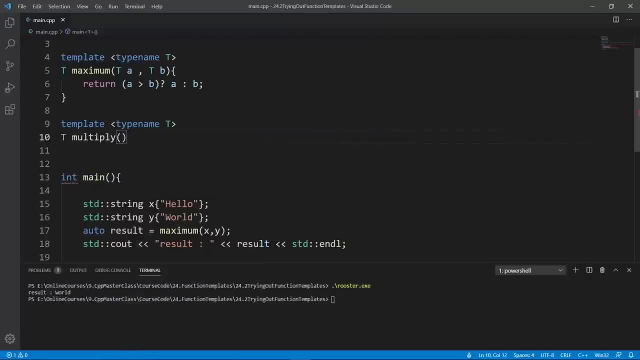 going to be the return value and we're going to say multiply, and we're going to multiply two parameters. we're going to say T a and T B, okay, and we're going to put in the logic and we're going to just return a multiplied by B. this is our multiplication operator in C plus plus, and we can. 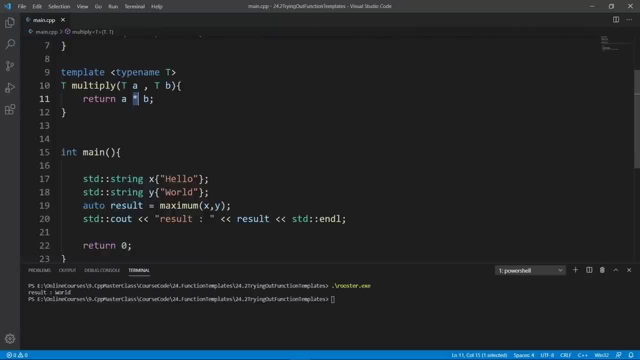 use this function. so, for example, we can say: we can comment this out and we can set up two variables. we're going to say and X and we're going to put in whatever we had before. let's put in five and and Y, we're going to say seven. I think this is what we used before. you can really put in whatever. 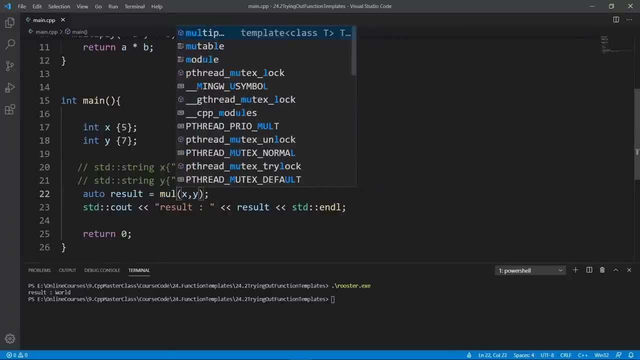 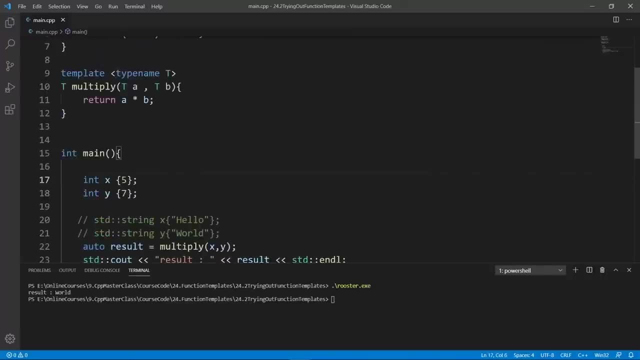 you want, and now we're going to call the multiply function template. so what this is going to do is to generate a function template instance which is going to be of type, and it's going to do a replacement here and replace T with and, and then we're going to multiply two and parameters that are passed to. 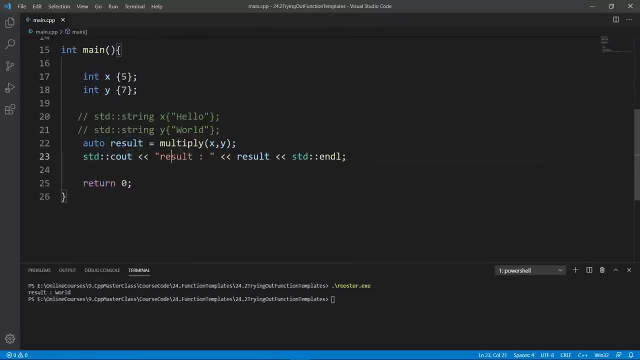 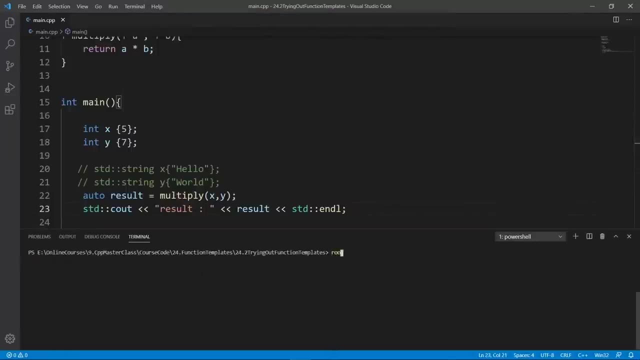 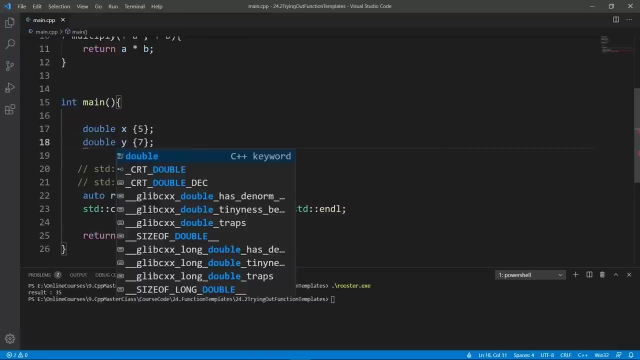 this function and we're going to return it and if we do that, we're going to get 35 printed out. let's prove this. we're going to use gcc to world. the world is good, we can clear and run rooster. we get a 35. if we change this to double, it is going to work. so let's change this to double and maybe 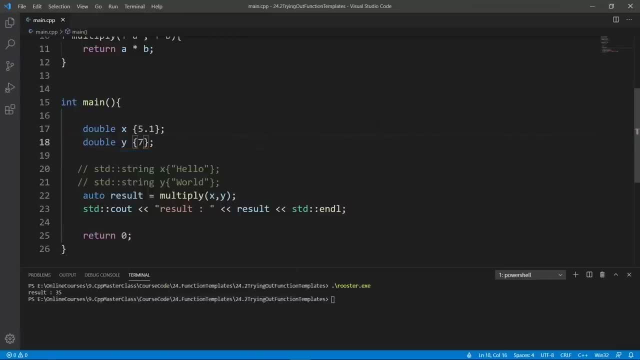 put in 5.1 and 7.0- why not? and then we're going to see what we get. we're going to build with gcc. the build is good. we can clear run roaster. we get 35.7. this is what we expect. but watch what happens if we try to use the std string types. okay, I want you. 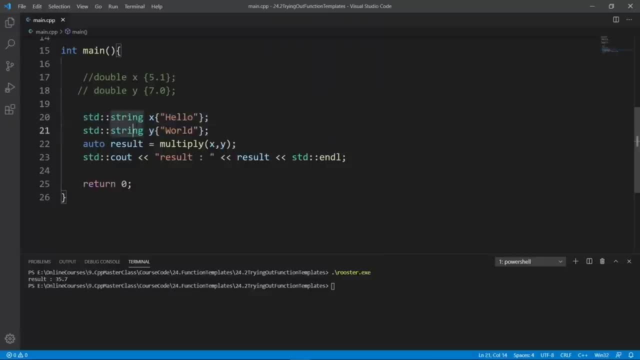 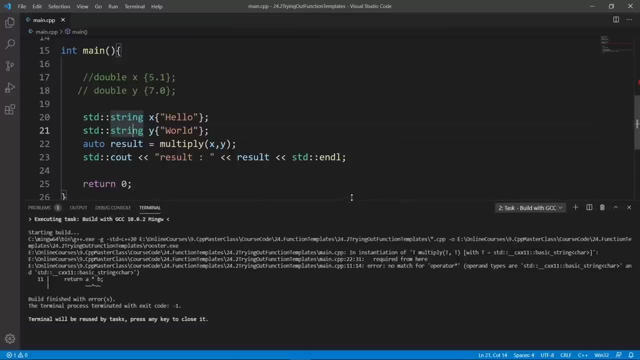 to see that. so we're going to enable our std string variables here and if we try to build, we're going to get a compiler error. but I want you to try and guess why. why do we have this compiler error? if we look at what gcc is saying here, it is saying: in instantiation of our function template required. 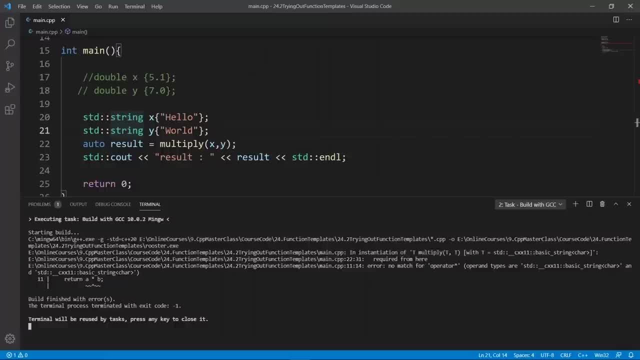 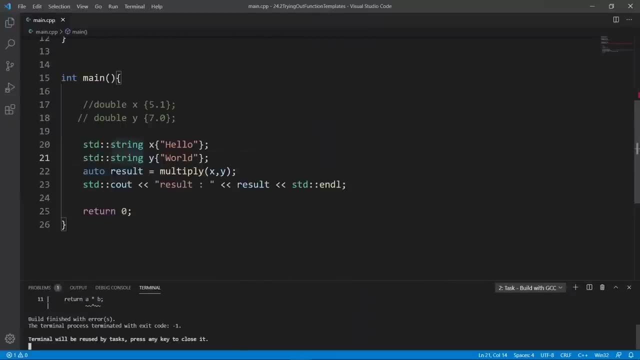 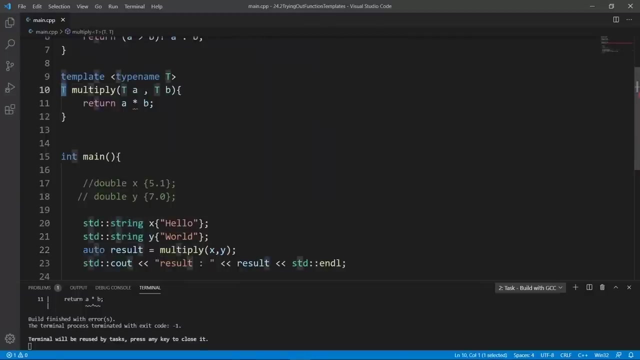 from here and no match for operator multiplication here. and this is the problem. the compiler is going to do what it knows to do. it is going to do a replacement in our function template and it is going to replace T by std string, because that's the type we are using as an argument here. the 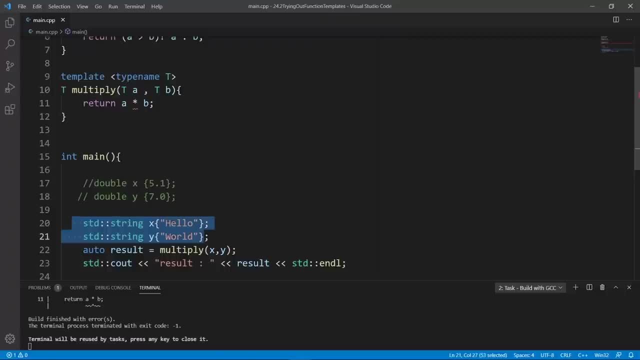 problem is we can't really multiply two strands. if you try to multiply two strings like we do here, it's not going to make sense. what do you expect to get if you multiply two strings? it doesn't make sense. the compiler doesn't know what to do with this operation. it's going to give you a compiler. 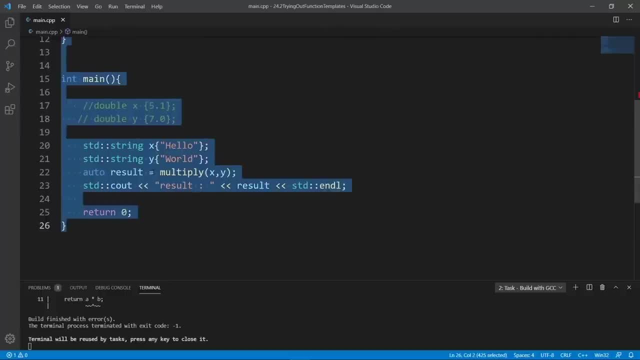 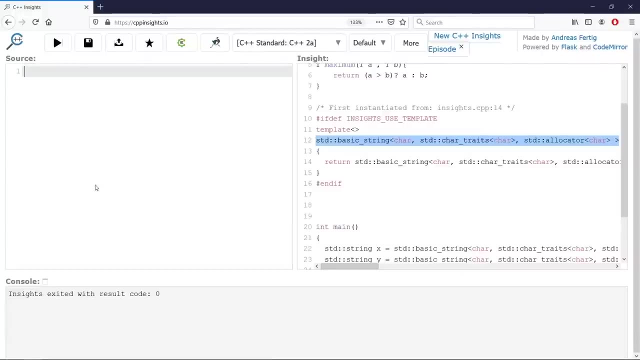 error. okay, to really drive this home, let's go back to cpp insights and put in the code here and see what is generated by the compiler. you should use these tools to your advantage because they really help in understanding what is going on. so let's hit the play button here. I just put in: 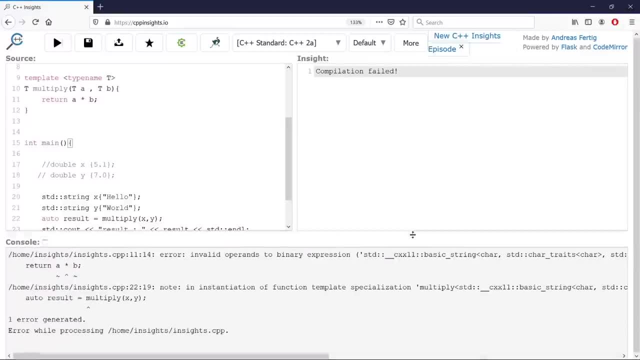 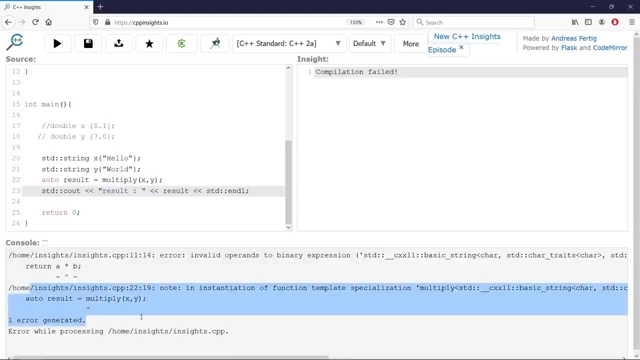 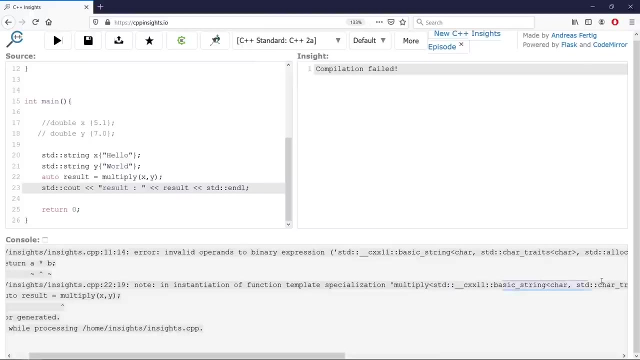 my code and it is going to say compilation failed because we have the same error. cpp insights needs to compile the code correctly to give you the template instantiations. but here you see that it is basically giving us the same error. let's try and see the entire thing here and see if we see. 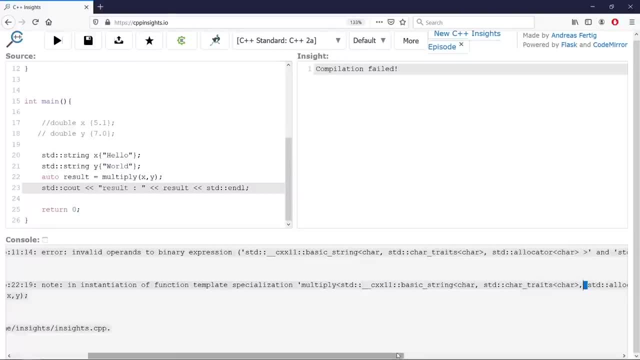 the real error and we can't really scroll around with us. I'm having trouble scrolling around here. I can use these buttons, I guess. okay, so let's see. if we see the actual error and we're not seeing it here, auto result: multiply: error generated. so we're going. 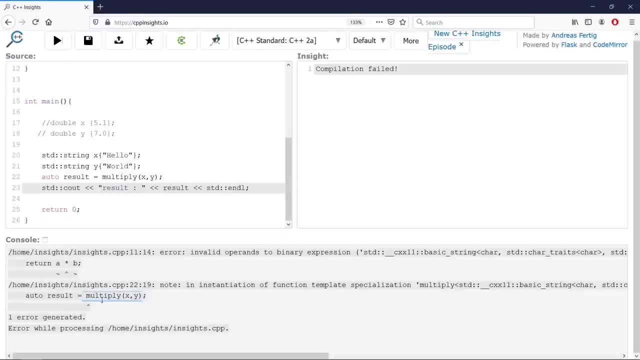 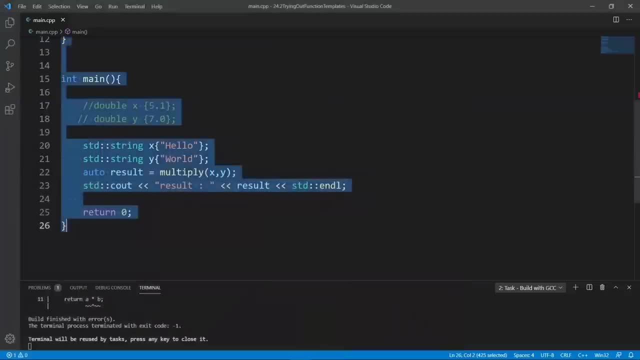 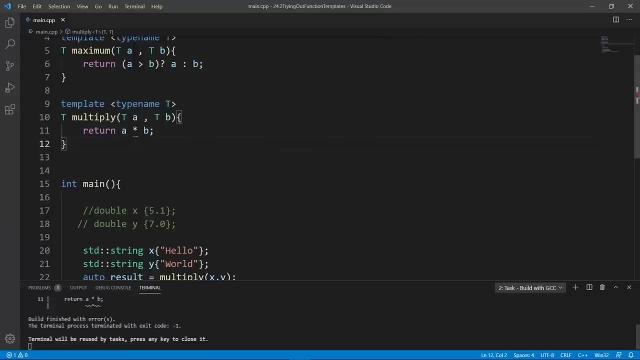 to get an error if we try to instantiate our template with the types that we are passing in here, which are std strand. cpp insights isn't really helpful here, but hopefully you understand the problem. the problem is if the compiler tries to generate a template instance using std strand. multiplying two strands isn't going to make sense, so the 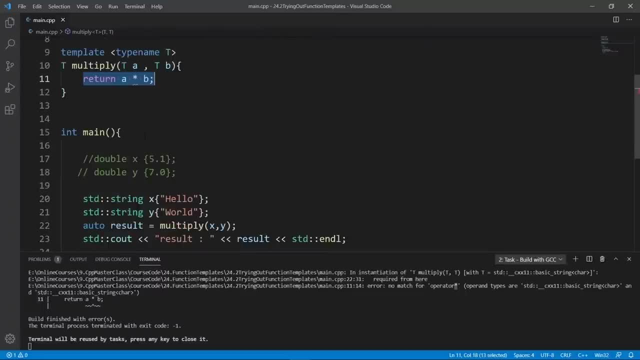 compiler is going to give you a compiler error because this is not supported. so the message here is that you should make sure that the template instances generated by the compilers support whatever operations you are doing in the body of your function template. this is the message here. another thing I want you to see before we close this off. I'm going to take out this. 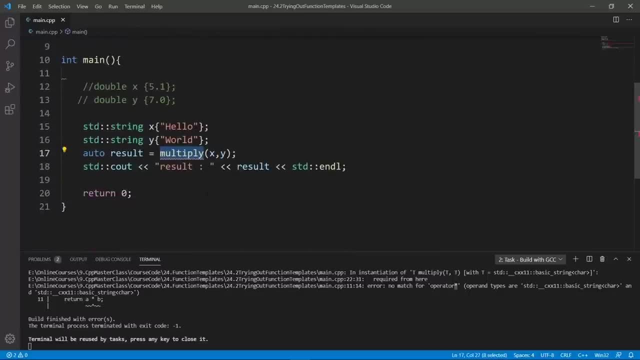 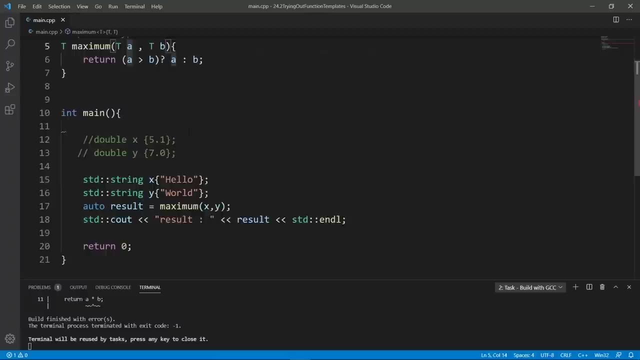 automatic line here and we're going to go back to our maximum function. what I want you to see is that if you pass different types for this function template, you're going to get a compiler error. and what do I mean by that? let's take out our std strength because it's no longer useful for 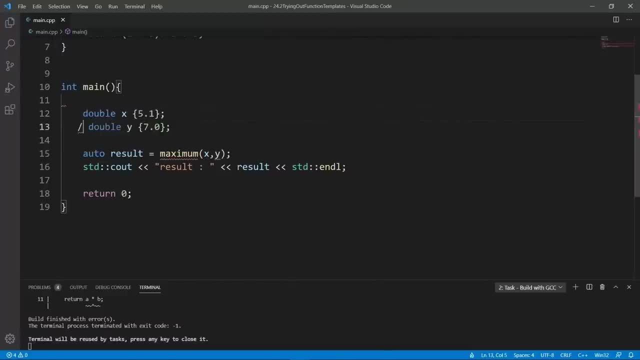 our purposes here and we're going to just use double and int parameters. let's use ant here and we make this an intellectual, our maximum function. you see that we have a squiggly line because the function template is forced to use the same type for the return type: the first parameter and the second parameter here. 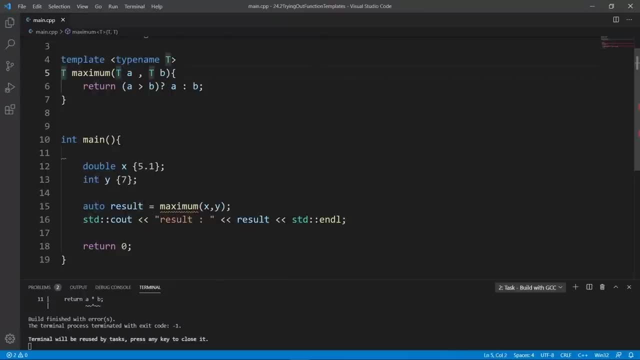 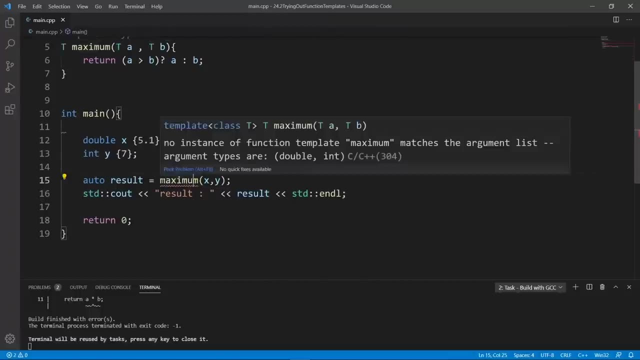 because the placeholder is the same. so the compiler is supposed to use the same thing for the first argument here, the second argument and the return type that we get from this maximum function here. but the problem is we are passing in parameters of different types and this is going. 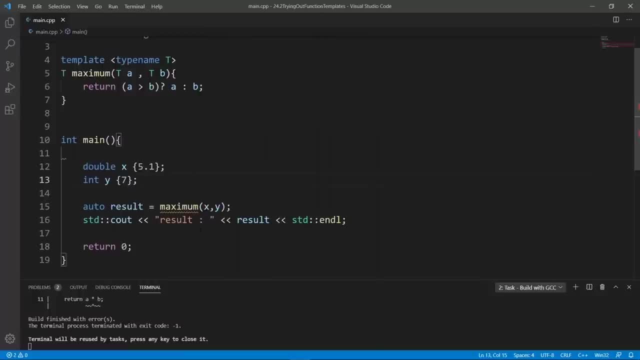 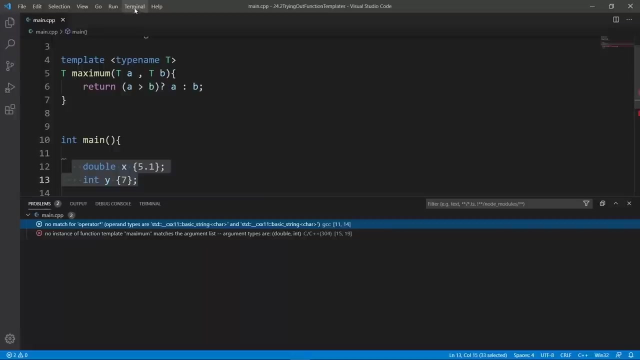 to give us a compiler error because the compiler want to know what to do with the types that you pass in as arguments. and if we look at our problems tab, here, visual studio code should give us an error: no match for operator. this is the error we had before. we can try and build again. 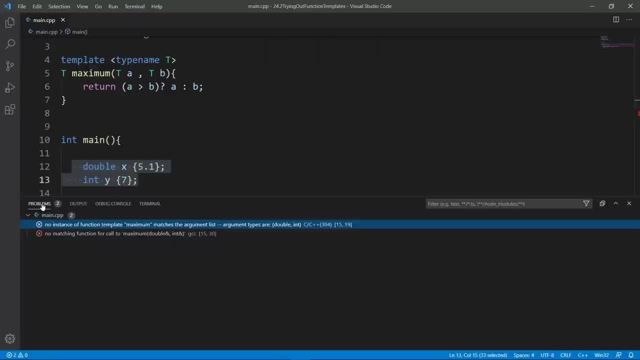 we're going to get a compiler error again, but this time it's going to be different. it's going to say: no instance of function template maximum matches the argument list that we are using, which is double and end. so this is a problem, but we will see ways around this as we. 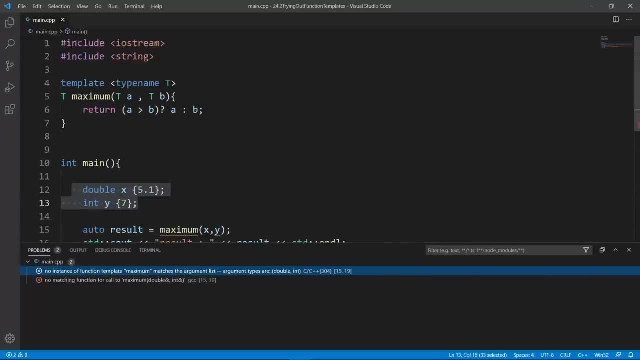 progress in the chapter. but what you should know is that if we set up a function template like this, this is going to enforce for all the types where we will place in t to be the same. if they're not the same, the compiler want to know how to do its replacement, and it is going to give you a compiler. 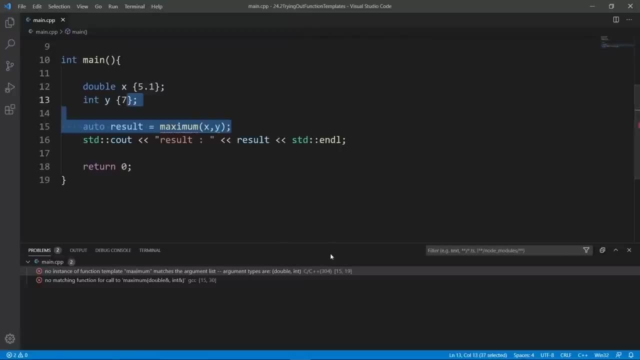 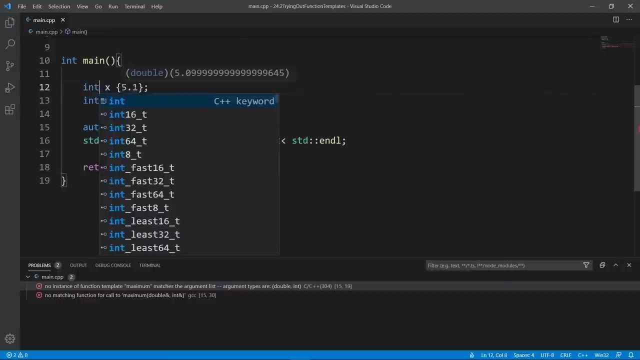 error. okay, the last thing i want you to see is that we can use the debugger to debug the function templates. so let's turn this back to end, because we wanted this to compile. so let's take out the decimal point here so that we have proper and literals, and if we compile again, this should. 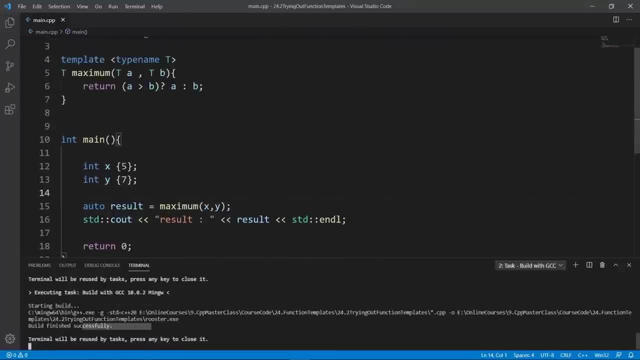 compile. okay, the world is good. now what really happens? if you try to debug a program with function templates, are you going to be working on the template instances? because, remember, the function templates are going to generate a function template and it's going to generate a function template. 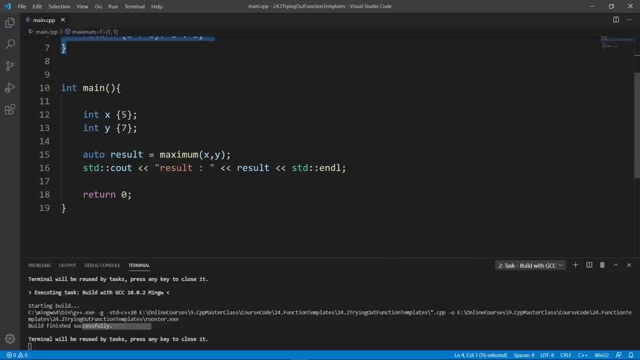 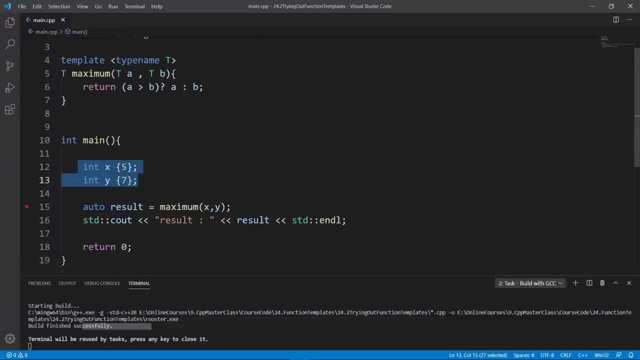 instances with actual types. for example, our template instance here is going to have ants because we are passing ant as argument here. so how are we exactly going to debug this? let's try this: we're going to set up a break point here on the call to our maximum function and we're going to 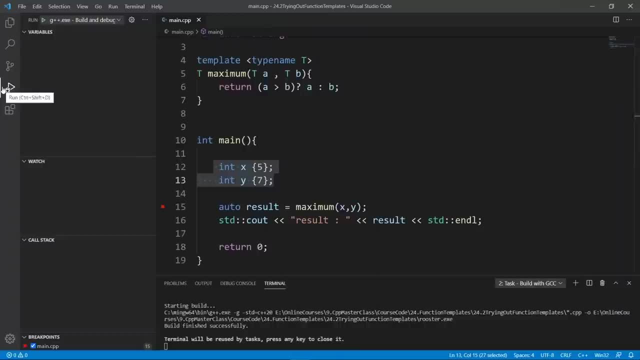 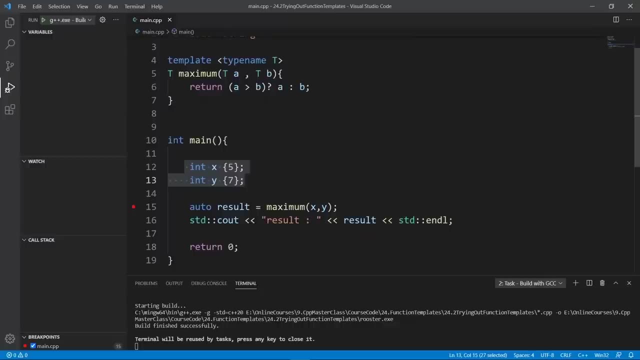 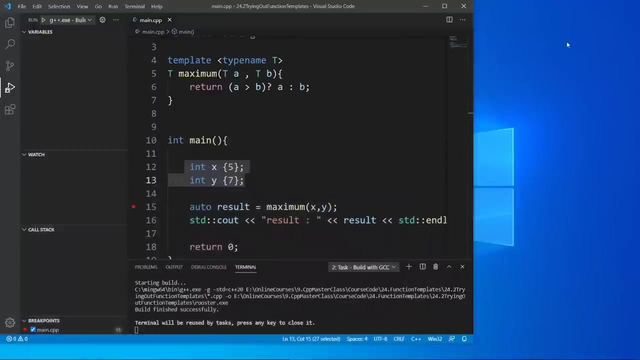 start debugging. we're going to go to our run tab here and we're going to use the debugging tools that come with gcc. see, we have seen how to do that in the last chapter and we're going to start debugging. let's minimize this guy here so that we have some breathing room, and we're going to run our debugger. 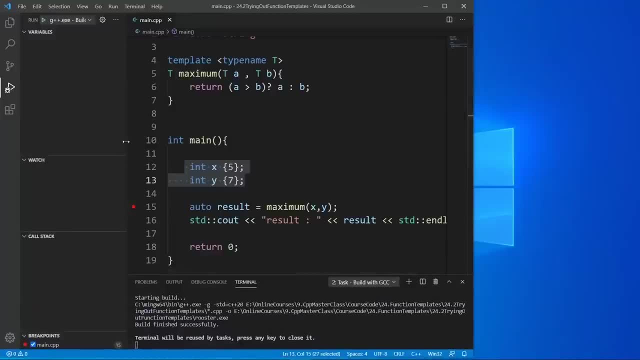 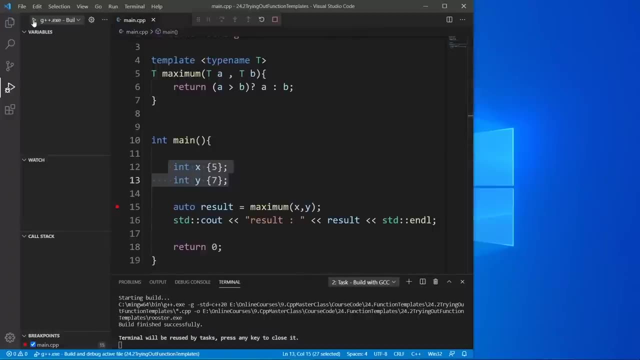 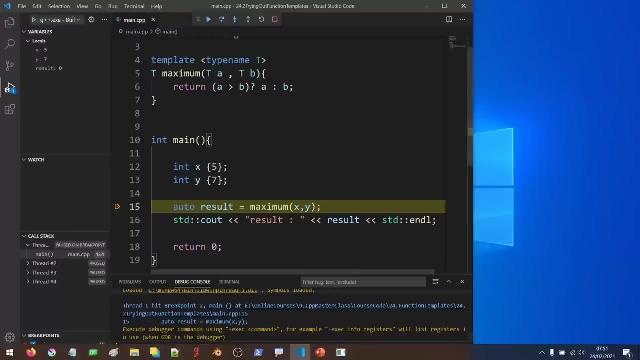 let's maximize this a little bit and push this a little to the left and we're going to start debugging and see what really happens here. so we hit the green button here, we're going to start debugging. our code is building now. the build is done. the binary has been passed to the 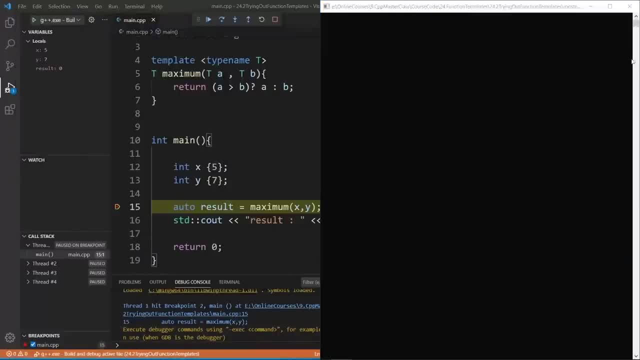 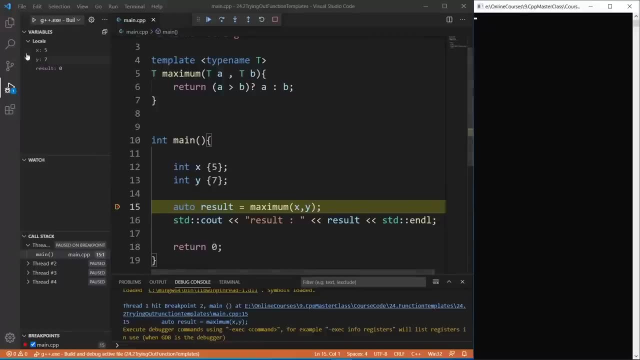 debugger, and now we have hit our break point here. so let's minimize this a little bit so that we have an easier way to save this. we have hit our break point. you see, the locals are what we have in the main function, which happens to be to the top of the call stack here. okay, now we want to jump into. 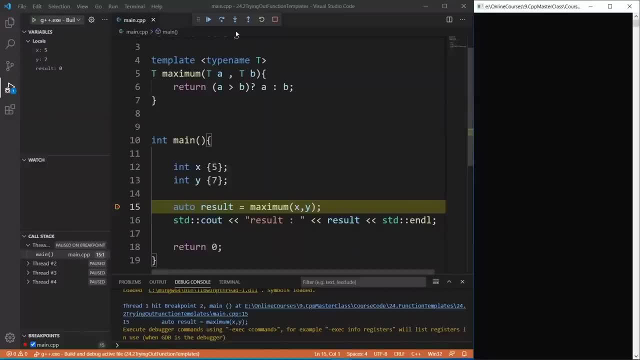 the maximum function and see the types that we have inside. so what we want to do here is hit the step into function and you notice it is going to jump into our function template here. but we're giving a function that's going to give you a function that's going to give us the types. 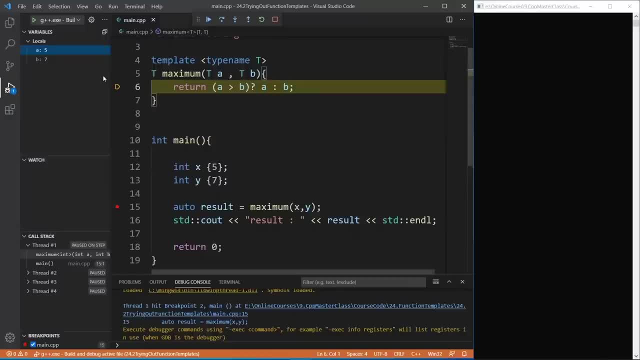 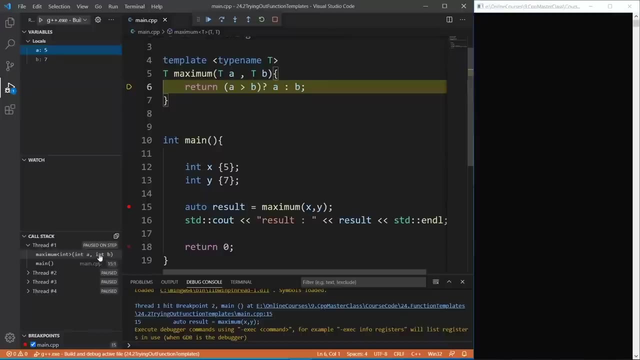 and this is because this is a function template. it's not going to give you the types because it's not easy to get those here, but if we look at the call stack, you see that we have information about the types of the function that is being called. we are calling int a and int b and it is going to. 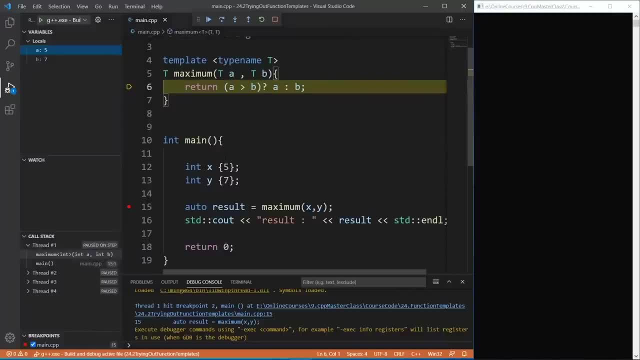 return and you see that in the angle brackets here and again. this is possibly another way to look at what template instances where it's going to return the function that we have inside and we're going to generated by the compiler, because we see the function called here is taking int parameters. 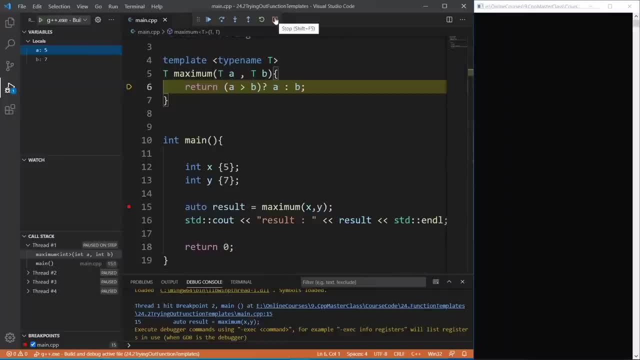 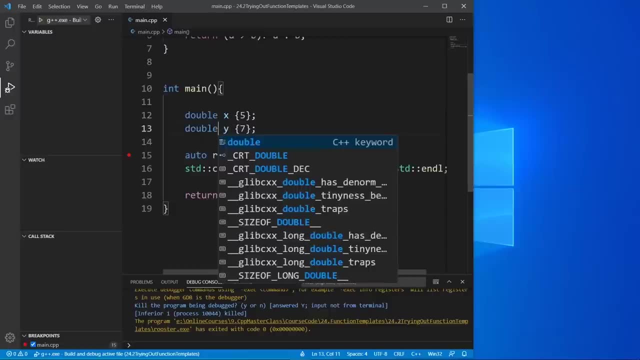 and it is going to return int. let's kill our debugger, because this is really all we want to see, and change the types to double here, and we're going to see that the function to the top of the call stack is going to be taking double parameters. so let's change this back to five point something. 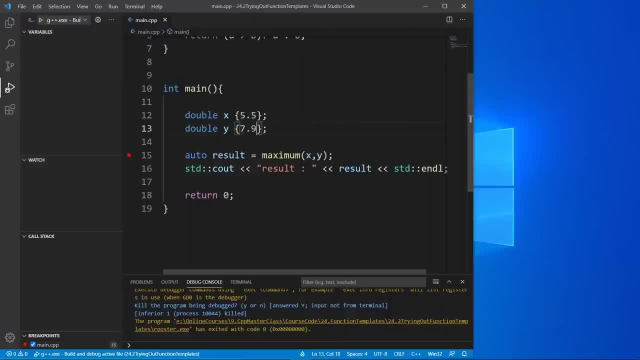 five, point five, maybe seven and point nine- why not? and we're going to print our results here. but what we really are interested in is seeing the function template instance generated by the compiler because of this call here, and we can do this through the debugger. this is a little bit. 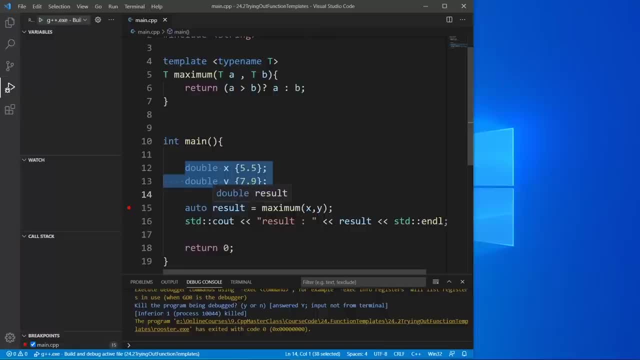 convoluted because you have to set up breakpoints and whatever, but it is helpful if you don't want to use things like cpp insights, as we have seen before and again. this is also useful because we're going to be able to do this through the debugger, so we're going to do this through the 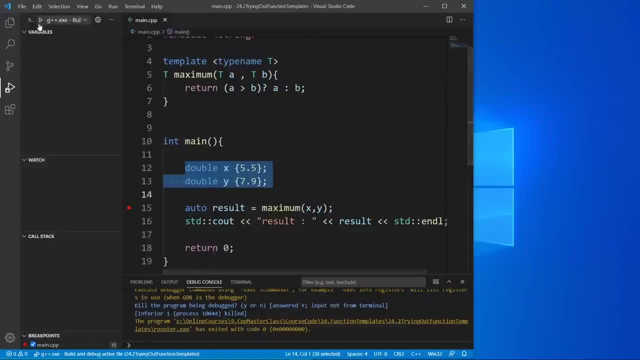 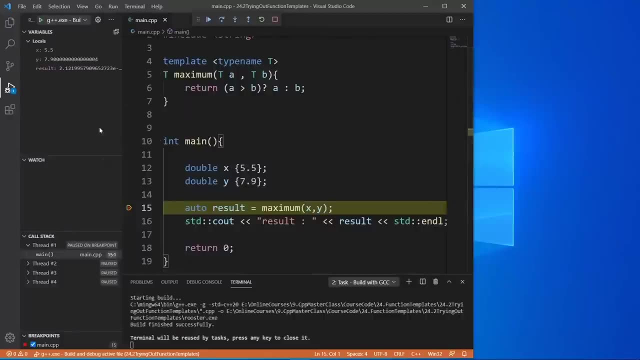 debugger, and we're going to do this through the debugger and we're going to do this through the. you will need to debug your code if it is using function templates. let's run this to really prove our point. here. the world is going to go through. the binary executable is going to be. 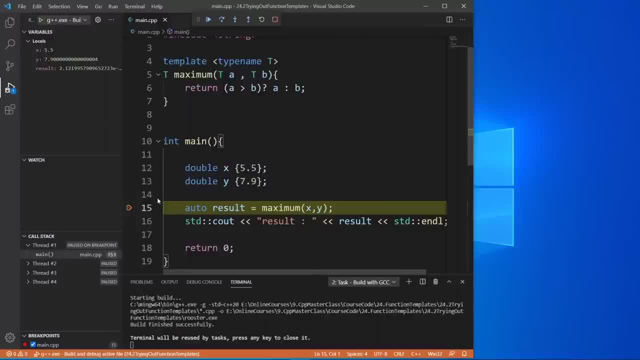 passed into the debugger and we're going to hit our breakpoint here again. you see, our locals are not giving us the types here, but we cannot use the function call stack to really see this. we have hit the breakpoint here at line 15, so we can step into the call and if we hit the body 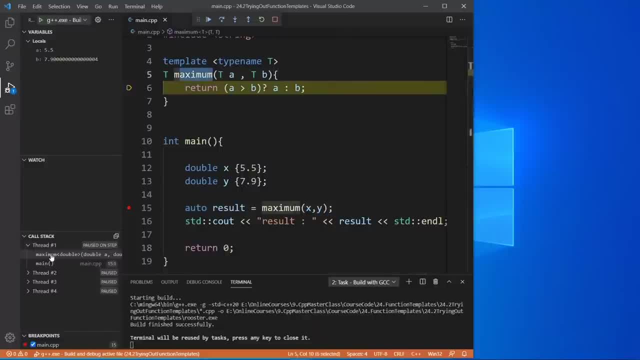 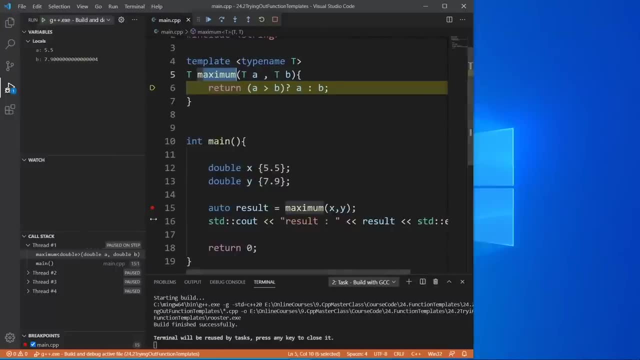 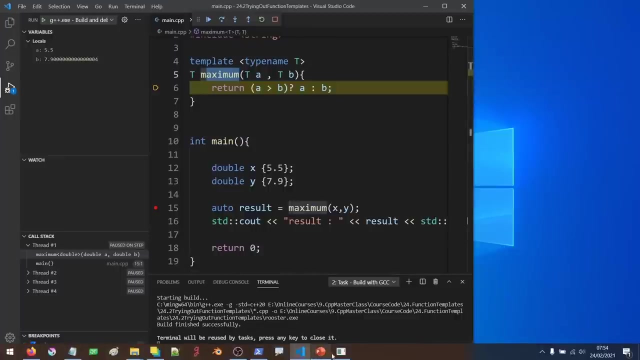 of the maximum function here and look at the call stack, we're going to see that the parameters we have in our function call are of double type and again, this hopefully proves to us that the compiler has actually generated a double function template instance. okay, since we are debugging, we can. 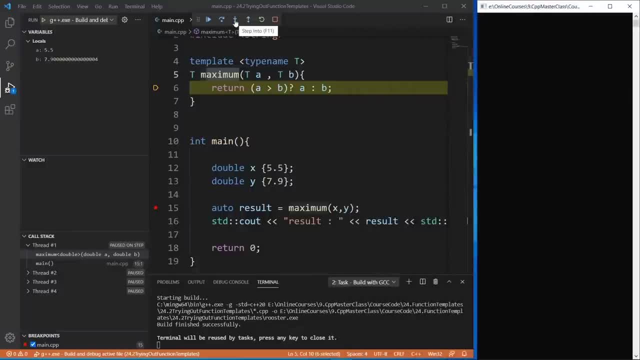 actually try and follow this program. let's hit next so that we can hit the end of this function. we can finish it and hit the main function. by the moment we hit the main function, result is going to be 7.9, which is what we have here and it is what we're going to print. we can just step over this. 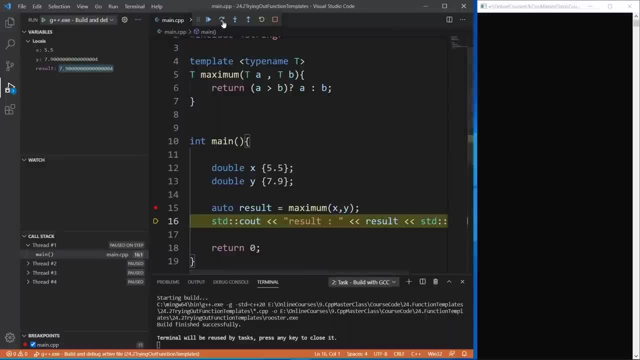 because we don't want to step into the logics of stdc out, so step over. we're going to print our result and our debugging session is going to basically end because we have hit the end of the main function. let's try and use the compiler from microsoft to see the information it. 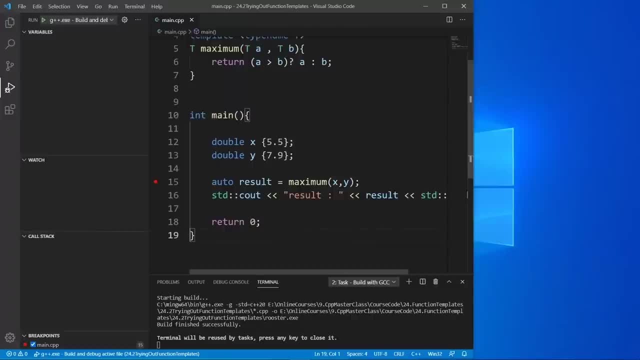 gives us, because these things can be different depending on the compiler and the debugging tools that you are using. we have the luxury to have these two set up here, so all we have to do is switch the tool we want to use here, and this is going to be using the one from microsoft, if you. 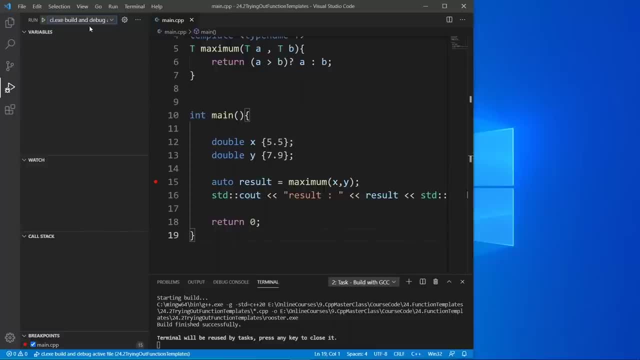 are not on windows or you don't want to use the compiler from microsoft and its debugging tools, you can just use gcc and its debugging tools here. i just want you to see different ways to do the things and that compilers and debuggers can give us different information. we're going to try and 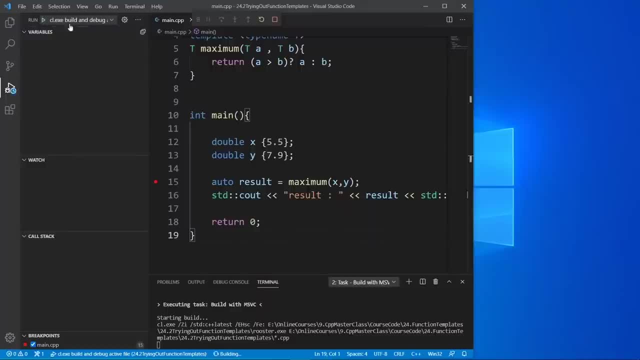 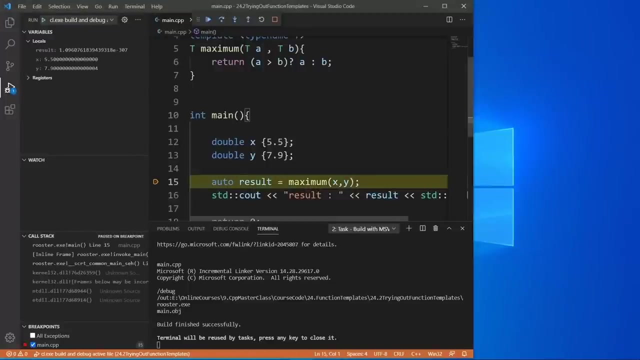 debug with this. so we're going to hit the green button here. notice that this is going to be using the compiler from microsoft. if we look at the build output here, you see that we are calling clexe. it is what we are using to build our binary. the binary is going to be passed to the debugger. 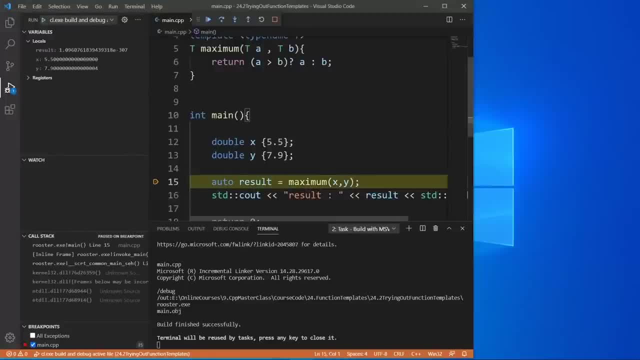 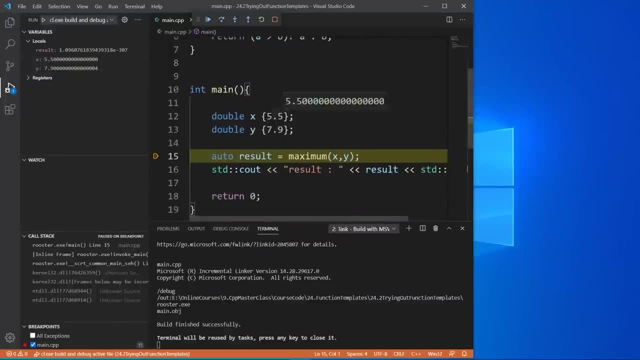 and then we're going to hit the breakpoint here, as we know, and then we're going to have our output here. these are our locals. you see, in the main function we don't see the types of our locals. why is that? i don't know why, but we see the values here in the main function and if we hit the step, 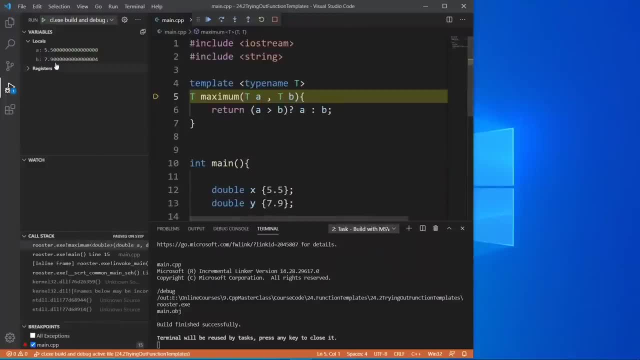 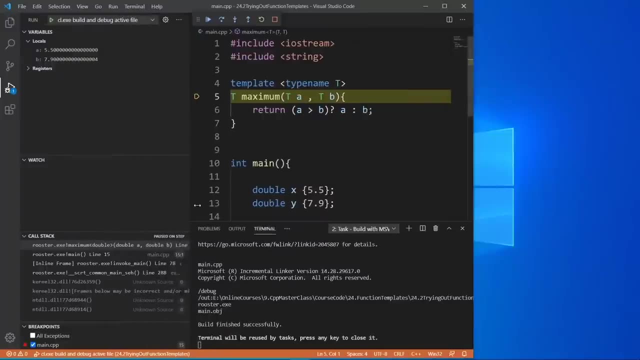 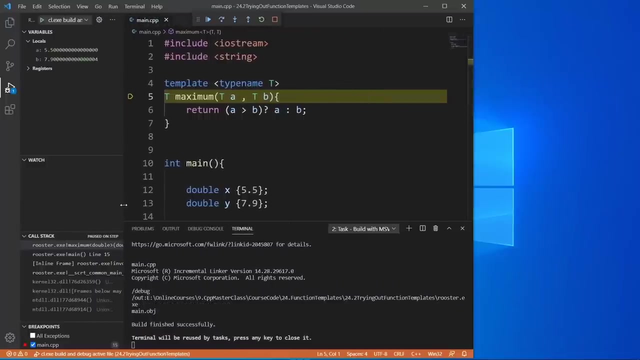 into button to jump into our maximum function. a is going to have this value, b is going to have this value and we look at the template instance, we can see the same information, but we are using a different compiler. this is really how you can debug your code that uses function templates, and this is going to give us a peek into the 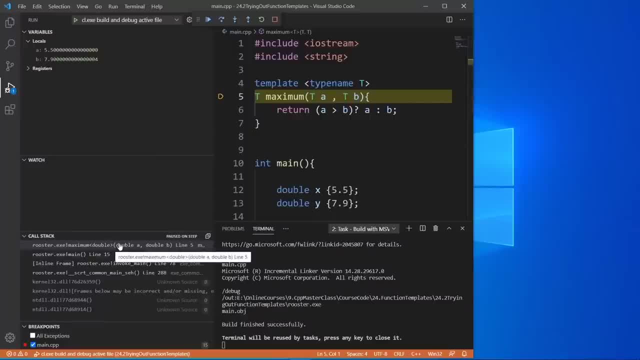 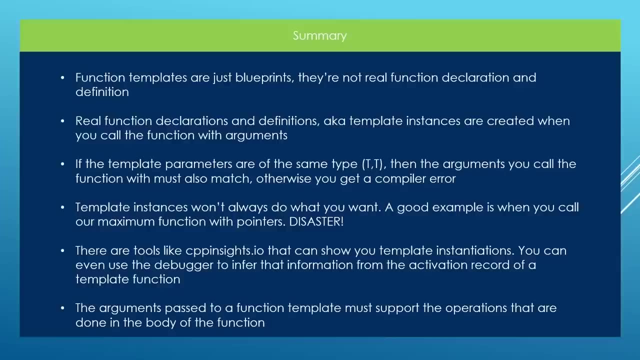 actual template instance that was generated by our compiler. this is really all i had to share in this lecture and before i let you go, let's summarize a little bit. function templates are blueprints. we have seen that the compiler is going to use those to generate actual 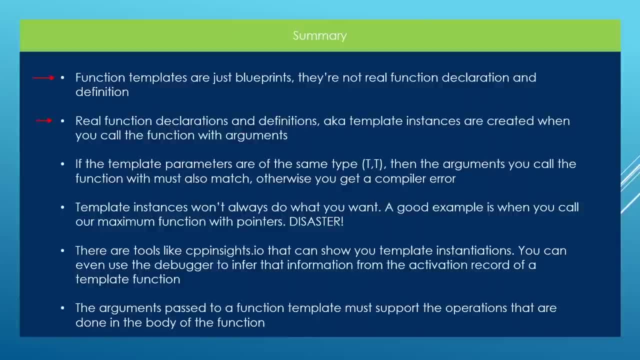 function template instances. real function definitions and declarations are going to be created when you call the function with arguments. if the template parameters are of the same type, maybe t and t, then the arguments you call the function with must also match, otherwise you get a compiler error. we have seen this, okay. here we have a point we haven't already covered: template instances. 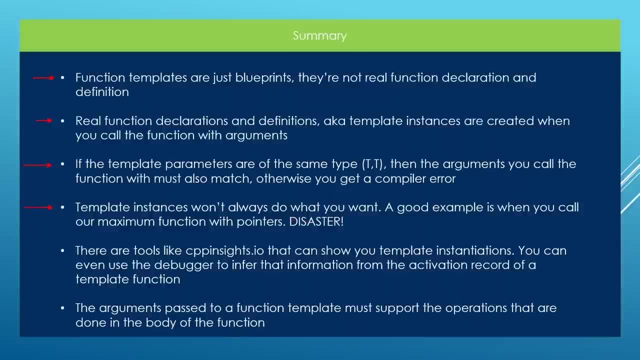 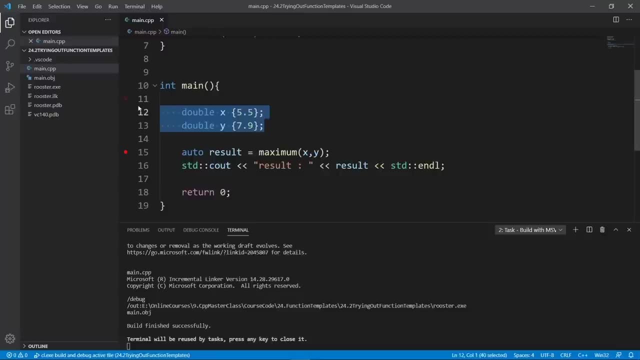 won't always do what you want. a good example is when you call our maximum function with pointers. so let's go back and really say this, because i want this to cover as much as possible about function templates. so let's go back to our code and we're going to modify things a little bit, okay, so what we're? 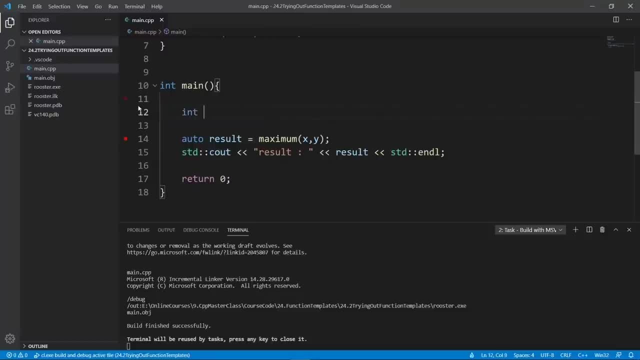 going to do here is take out whatever we have here. we're going to set up into variables x and y. x is going to be 5, as we have seen before, and y is going to be 7.. let's use this, and then we're going. 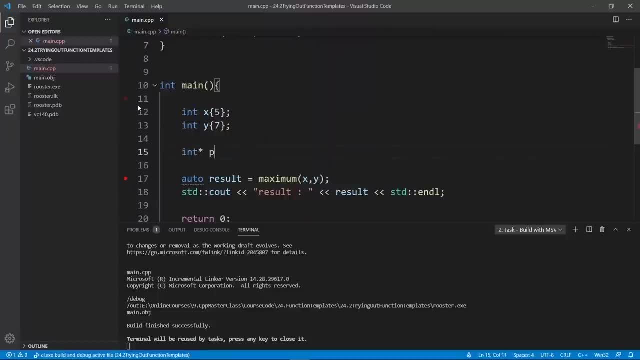 to set up two pointer variables. we're going to say end pointer px and we're going to initialize this with the address of x. nothing sophisticated so far. and we're going to say and py, and we're going to initialize this with the address of y. we can do this. the problem is going to come when we try to. 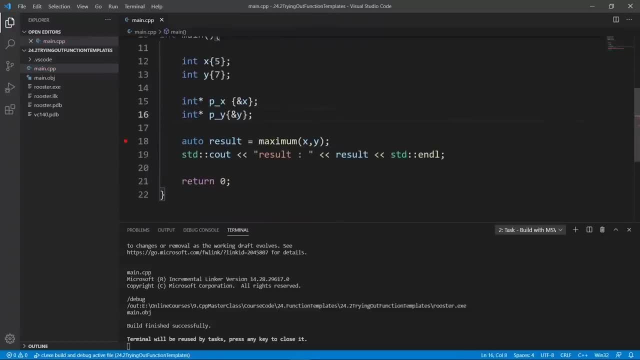 call our function here with the pointers. let's use px and py to call this function and py, and what this is going to do is to generate a template instance that takes end pointer. this is what the compiler knows to do. we're going to take the types that we pass in here which happen to be end pointer. 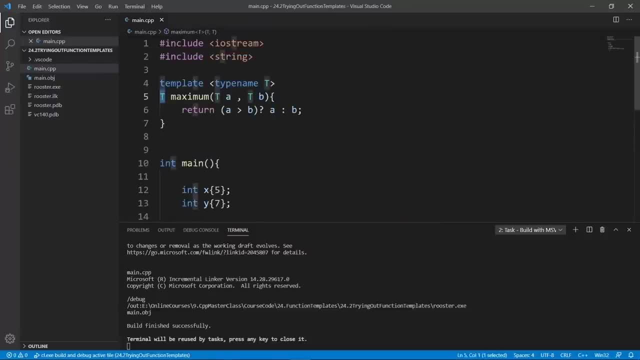 and we're going to change the return type to end pointer. we're going to change the first parameter pointer, the second parameter to end pointer and we're going to compute the maximum. if we compute the maximum here, we're going to be comparing pointers. okay, notice this. and if we try to do, 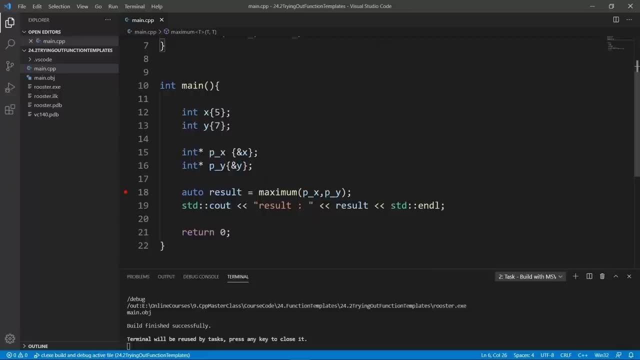 that we might not get what we want, because what we get now depends on the address used to store these guys in memory. hopefully you can see that and let's try and debug this program so that you can really see this. we're going to use the tools from g plus. 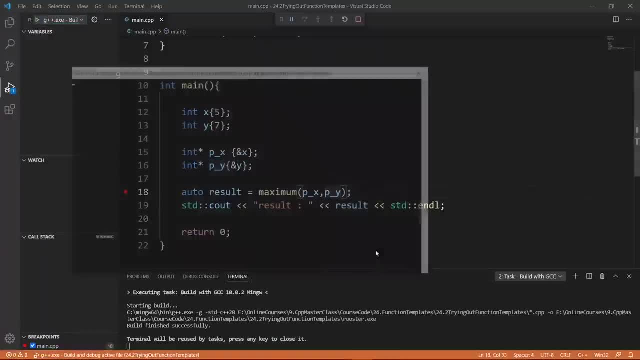 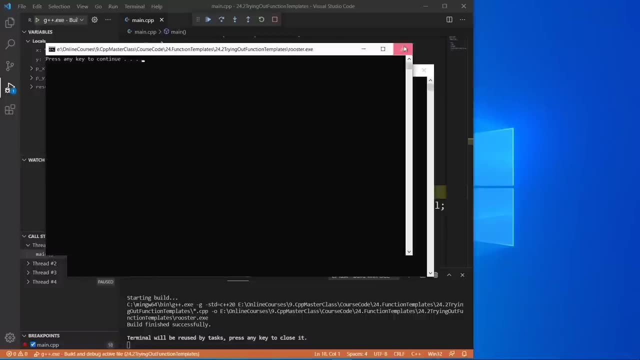 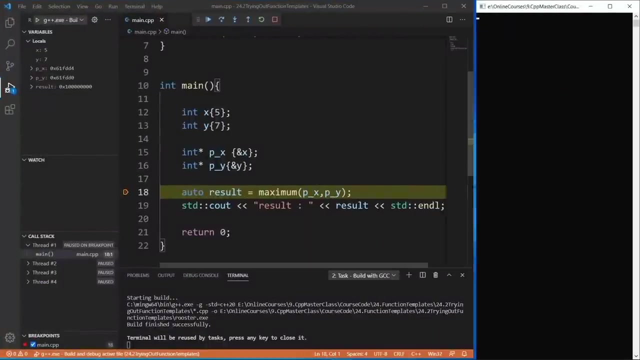 plus or gcc, and we're going to try and debug it. let's do that. it is going to run through the debugger and what we're going to have is our terminal here. i think this is not needed anymore, so let's put this to the right here and minimize a little bit. and now you notice that px contains: 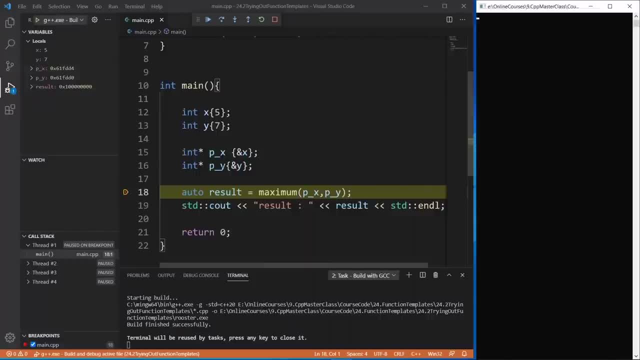 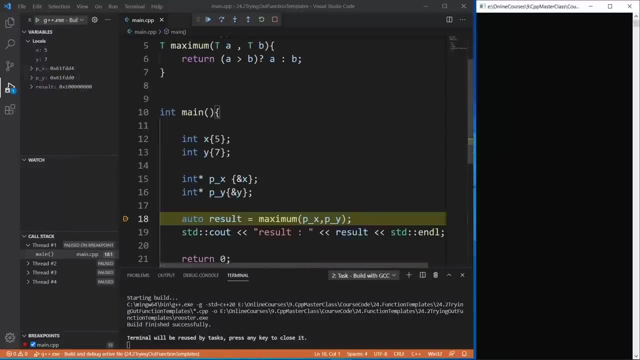 an address and py contains an address. hopefully you can see that in the body of our template instance we're going to be comparing these addresses, because we compare what we pass by a value here and what we pass are these two addresses. so whichever is the maximum in? 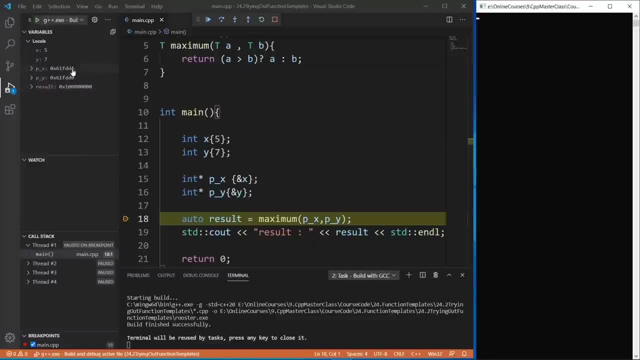 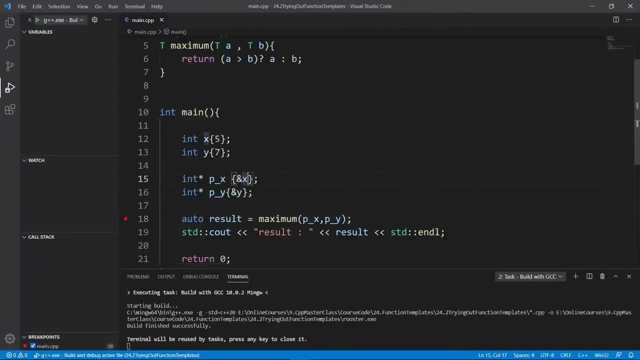 these guys and i think that's going to be dd4 here. it is the maximum. so whatever is contained in px is going to be considered the maximum. let's kill this because we have seen this information. so if we have a value in px and that happens to be at a bigger address, it's going to be considered. 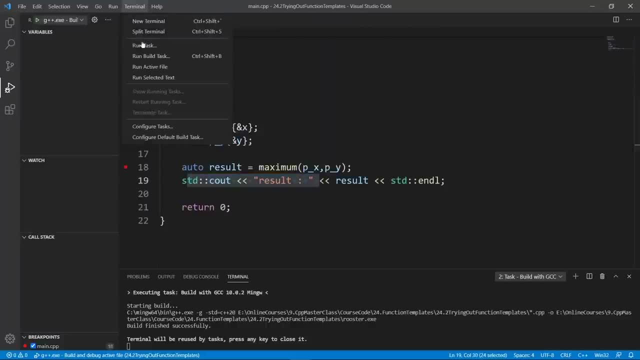 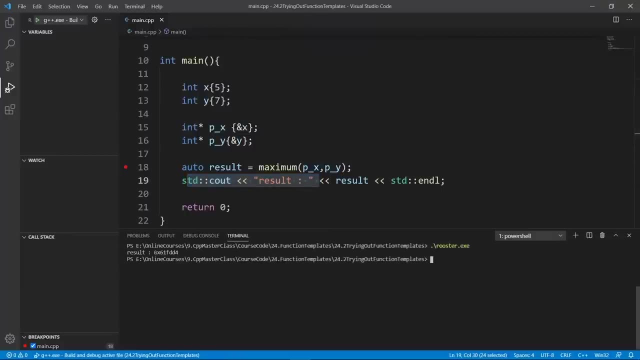 the maximum. let's see what we print. if we run this program, we're going to be building with gcc. let's do that. the build is good, we can clear and run rooster. now you see, result is some address, because we are returning a pointer and printing that out. but we can easily 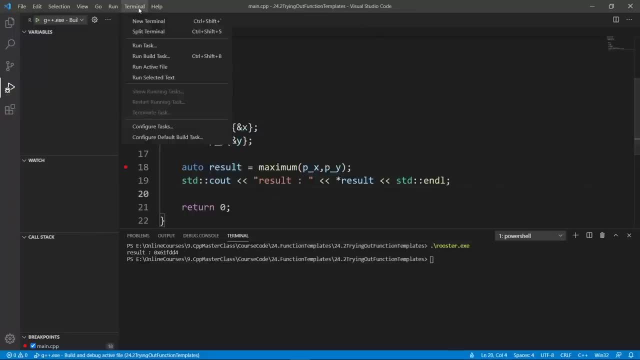 dereference this and get to the value inside this pointer. let's build again. we can clear and run rooster. this is going to give us result is 5 and hopefully you can see that this is really bad and not correct. we are trying to compute the maximum between. 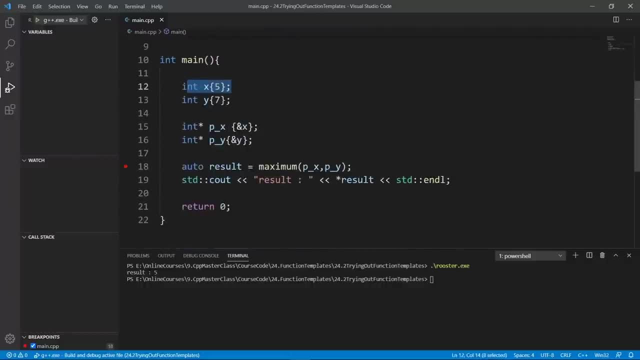 x and y and we are seeing that the maximum is 5.. so how can 5 be the maximum between 5 and 7? the problem is, we're not comparing the values here. we are comparing the addresses stored in these pointers, because that's what we are passing here. hopefully you can really save this. 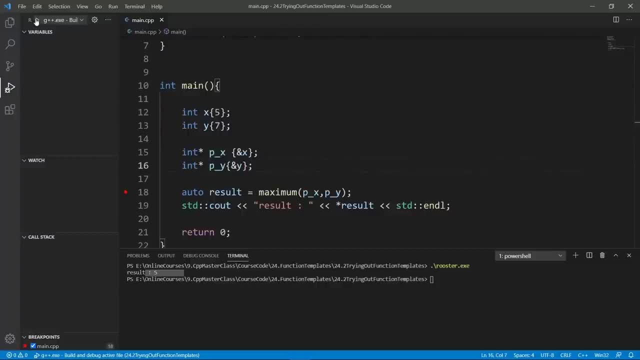 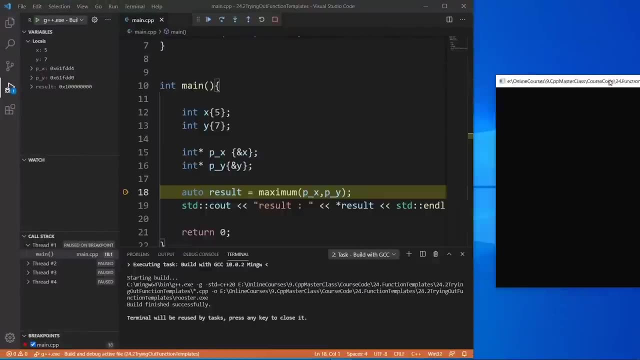 and we can prove this again through our debugger. we can run this through the debugger. we're going to hit the breakpoint- let's minimize this so that we can see our terminal window here- and we're going to move this around a little bit and now we have hit our breakpoint. if we 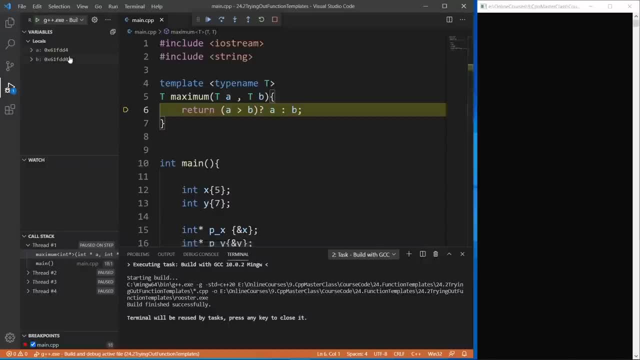 hit next to jump into the function. you see that what we are really comparing are a and b here, and a contains a much larger address, so it is the pointer that is going to be returned, and if we dereference that, we're going to be dereferencing the pointer that contains this x. 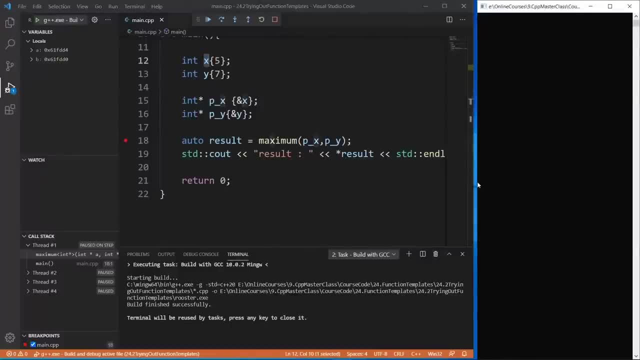 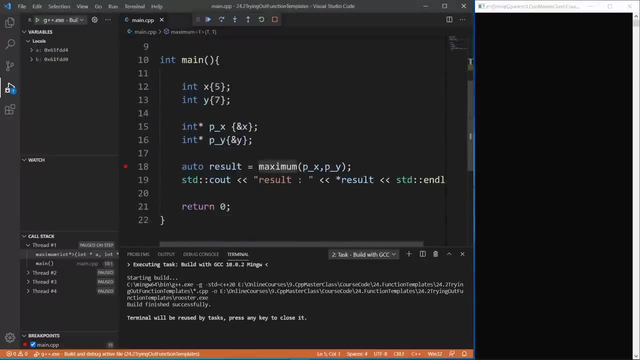 value and the message here is that you should be careful that your function templates are really what doing, what you want. somebody might do this if they are not careful, just passing pointer and expect to get the maximum, but the compiler is just going to compare pointer addresses and you're. 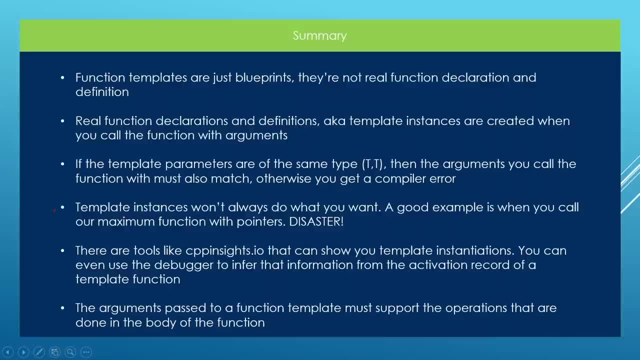 going to get something you probably don't expect. okay, this is what is meant by template. instances won't always do what you want. a good example is when you call a maximum function with pointers, you're going to get a wrong value. possibly there are tools like cpp insights which can show the 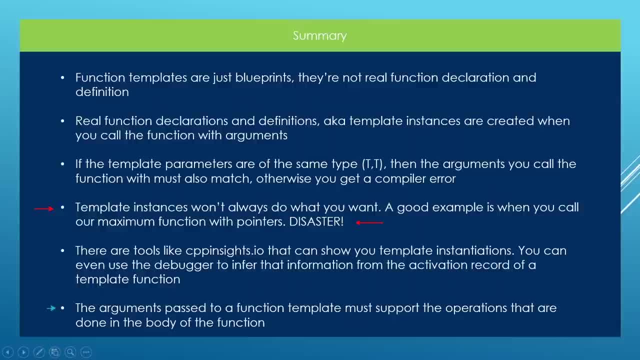 template instantiation. we have seen in the video of the template instance. we have seen a little bit of a way to do this, but we have seen that. and again, the arguments passed to a function template must support the operations that you are doing in your function template. we have seen an example of this. 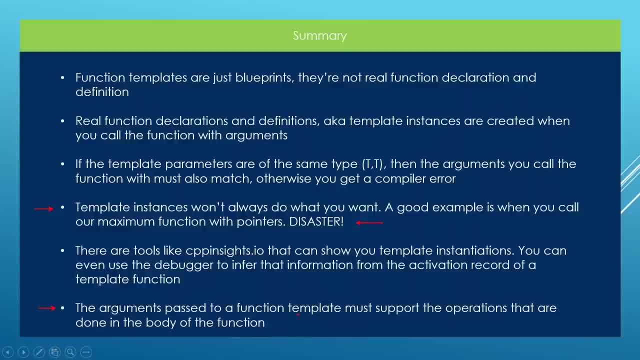 by setting up a multiplication function template and we saw that we had a compiler error if we try to pass std string arguments because we can't multiply two strings. this is really all i had to share in this lecture. i apologize, it turned out to be lengthy, but i really had to put this in one. 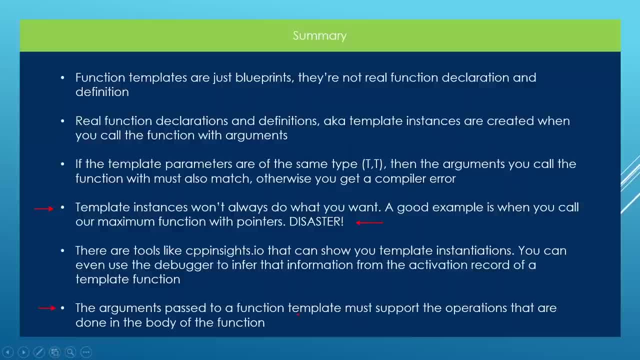 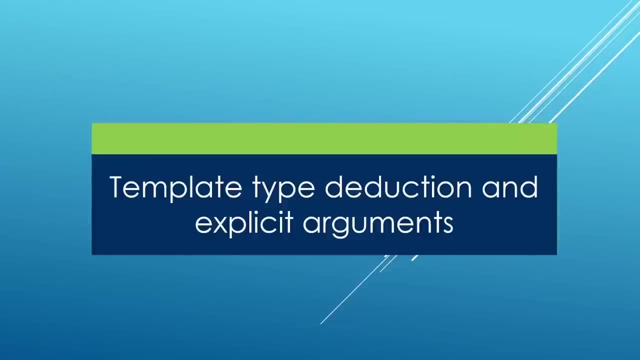 really show you different sides of the same things. we are going to stop here in this lecture. in the next one, we're going to learn about template type deduction and explicit arguments. go ahead and finish up here and meet me there. in this lecture, we're going to learn about template type deduction. 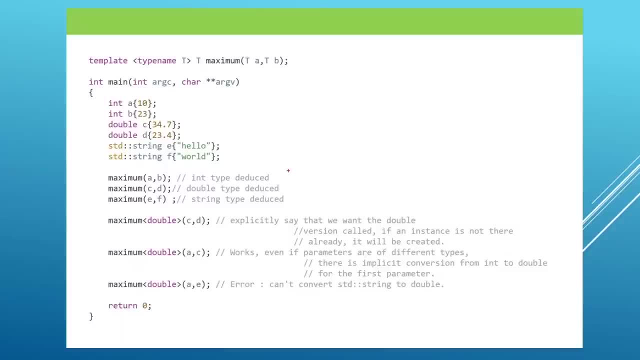 and explicit arguments. what we mean by template type deduction is the mechanism the compiler uses to deduce the type it would use to set up our template. instance from the arguments that we pass to our function call. here, for example, the compiler is going to look at a and b here in our call to the maximum function. 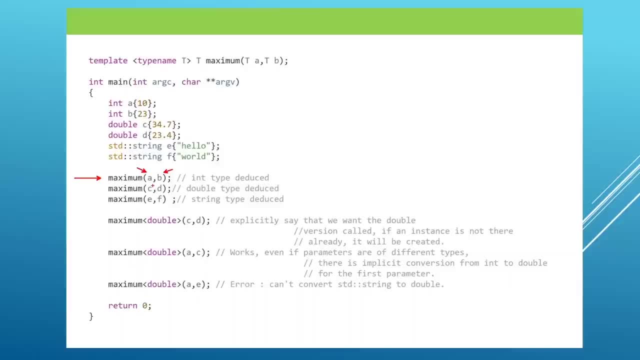 and it is going to notice that they are of int type. and then it is going to say: okay, you are calling your function with int types and i see that your function templates takes three replacers in here. so i am going to replace these guys with and, and it is going to guess that 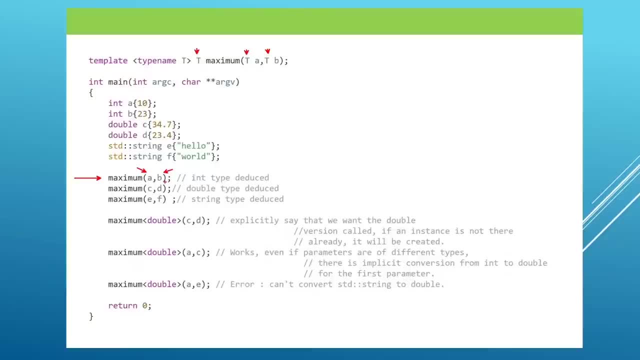 that from the call that you make here, there's no other mechanism to help the compiler out. this is really what template type deduction is about, and for the first example here we are passing in int parameters, so and is going to be deduced. for the second function call, 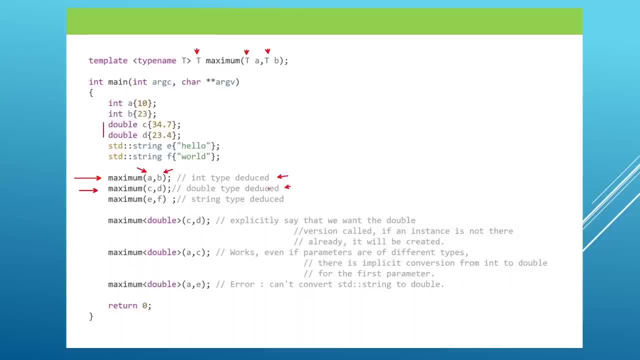 we are passing in double parameters, so a double function template instance is going to be generated for the third call. here we are using std string parameters, so we are going to deduce template instance that uses std string here. this is what we mean by template type deduction, but we 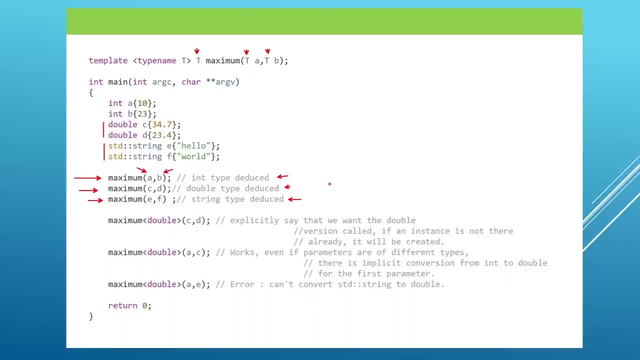 have seen that automatic template type deduction can really have problems, especially if you pass parameters of different types. for example, if we call our maximum function here with a and c, which happen to be int and double type, then we're going to have a problem because this function template. 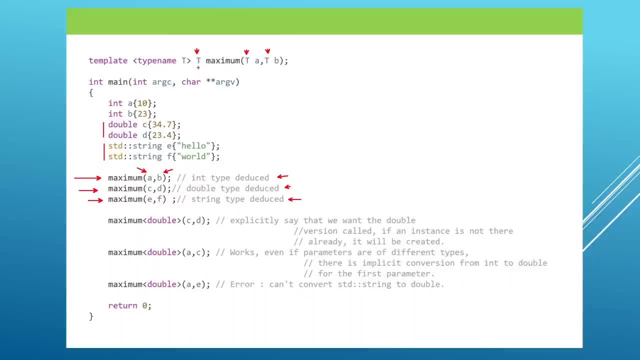 can't handle parameters with different types because the replacer is the same. the compiler is going to enforce that all the template arguments are of the same type and the template arguments are going to be what you pass in here. so a and b must be the same, if they happen to be. 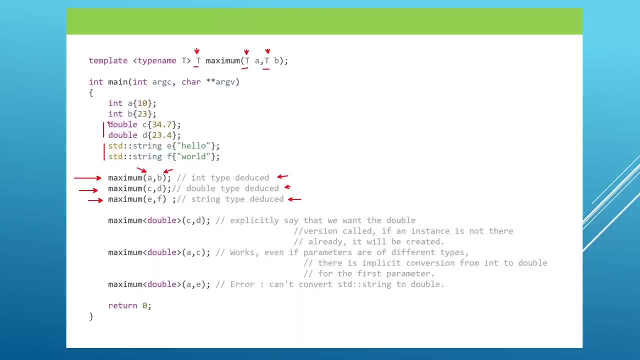 not the same. for example, int and double, you're going to get a compiler error. now we're going to see that we can use explicit template arguments and again i want to make it very clear the difference between the two types of arguments that we have in the template type deduction. 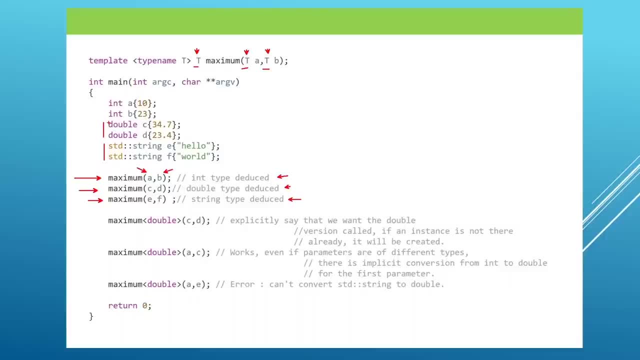 between a template parameter and the template argument. a template parameter is what you have in your function declaration or a definition. so what we have in our function setup here are template parameters. ta here and tb are template parameters, but what we have when we call our function template is going to be template arguments. for example, c and d here are template arguments, and 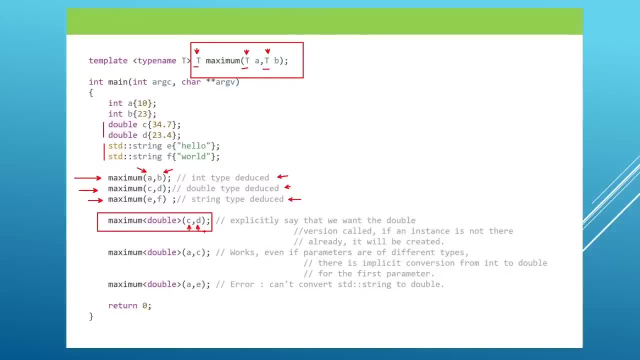 we're going to be using this terminology in this chapter and many more chapters to come in this course. make sure this is super clear. so what we're going to look at is using explicit template arguments, and what this means is a mechanism through which you can force the compiler to use some type to. 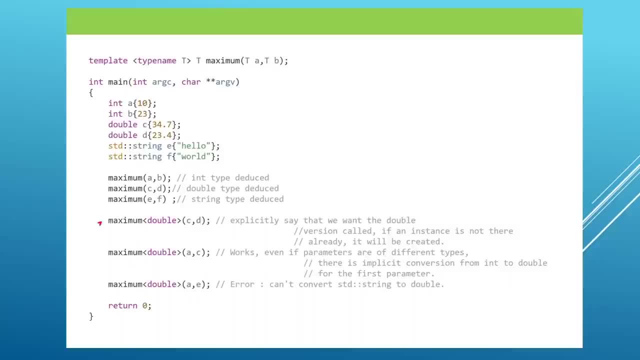 generate your template instance, and the syntax to do this is really simple. it is what we have here. we say maximum and we put the type we want to use to generate our template instance in the past, and then they look at our previous, for instance, and they say that the type we're using, which one we want? 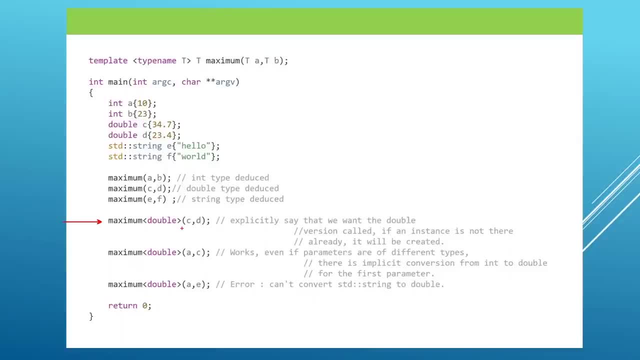 instance, in angle brackets, like we see here. so this is going to use double, so this is going to explicitly tell the compiler we want the double version called and it's going to generate that and that's what is going to be called by this call we have here. a good benefit with this is that now 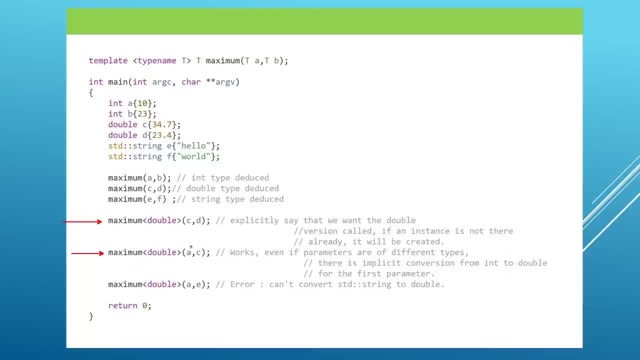 this is going to support template arguments of different types. so if we make the call like this, the compiler is going to see that, uh-huh, we are calling with int and double types because a is int and c is double, but it's going to see that you want the double template instance generated. 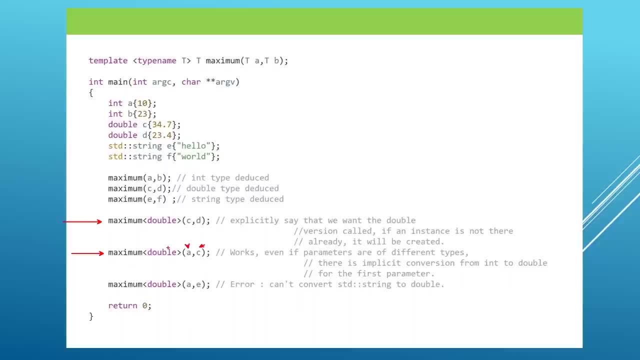 now the compiler will have the possibility to do implicit conversions from other types to double, and if this implicit conversion fails, then we're going to get a compiler error. so if you look here, for example- this is the example for that- we are passing in a and e and a is int and e is an std. 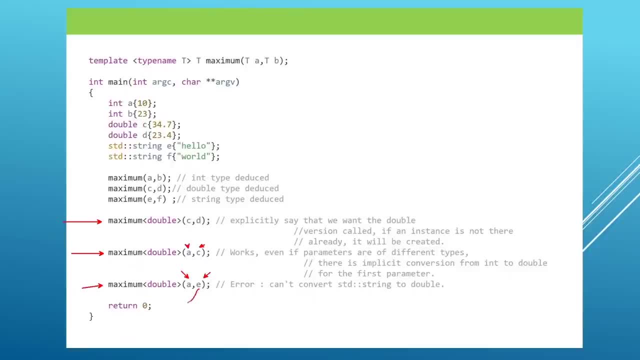 trend. we cannot do that in the compiler, so we are passing in a and e and a is int and e is an std, an implicit conversion from a studio strength to double. so this is going to give us a compiler error and this is really all template type deduction and explicit arguments are about. we can use these. 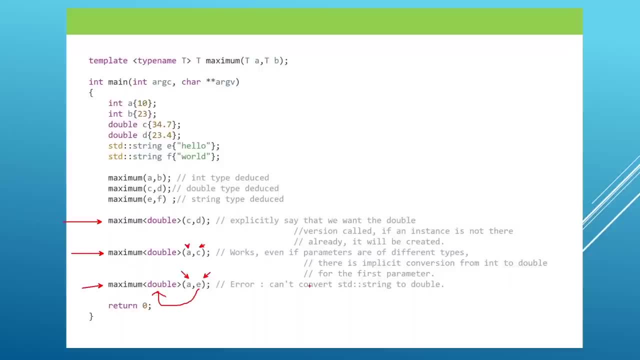 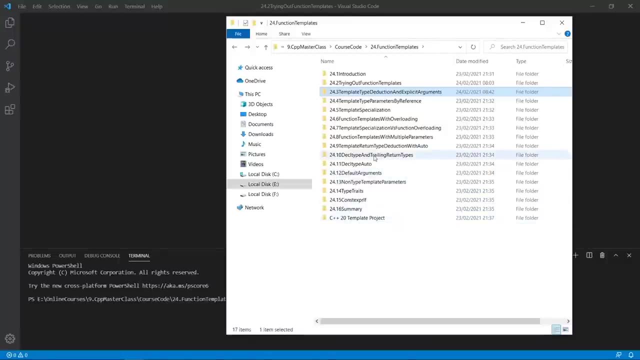 things to really make our code easier. now that you have this understood, we're going to head over to visual studio code and play with this a little more. here we are in our working directory. the current project is template type deductions and explicit arguments. we're going to grab our 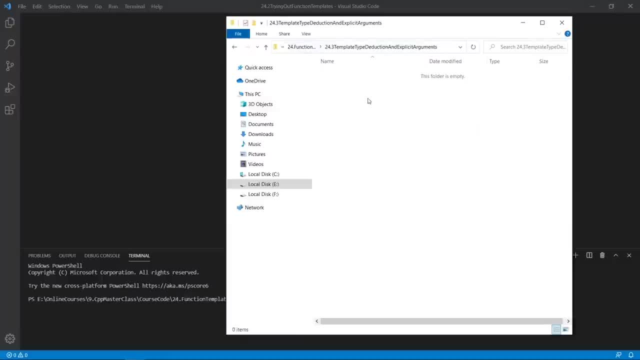 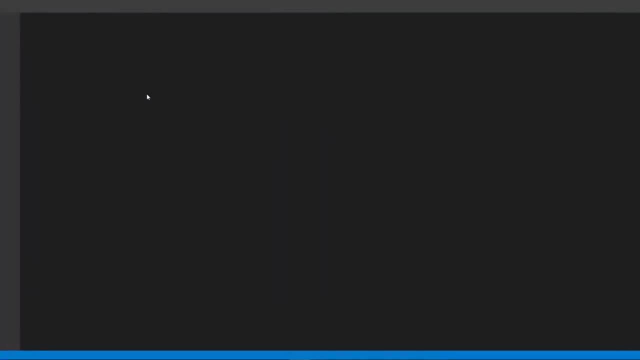 template files pretty quick and put them in place, and after that we're going to open this in visual studio code. let's drag and drop on top of visual studio code here. this is going to open our folder and we can open our main cpp file and set up our function template. let's clean this up a little bit. 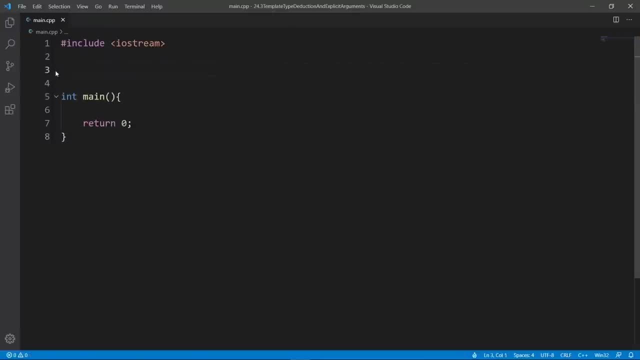 and we're going to set up our function template. let's type this out just to practice. so we're going to say template and we're going to say type name and we're going to say t and, if you want, you can put this on a single line, but i prefer to put this on separate lines. but 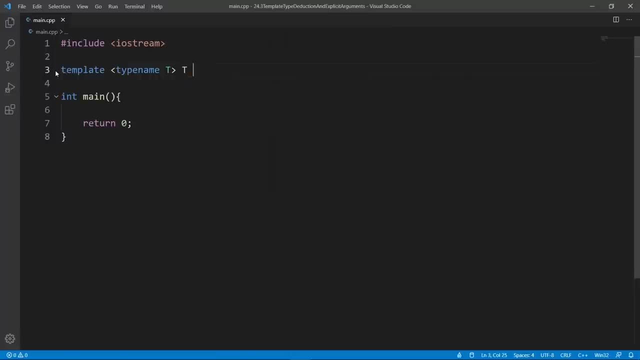 let's show you that. so we're going to say t here and we're going to say maximum and we're going to say the parameters. they are going to be of type t and we can pass them by value, just for now, and after this we're going to go in the body of our function template and then we can return whichever. 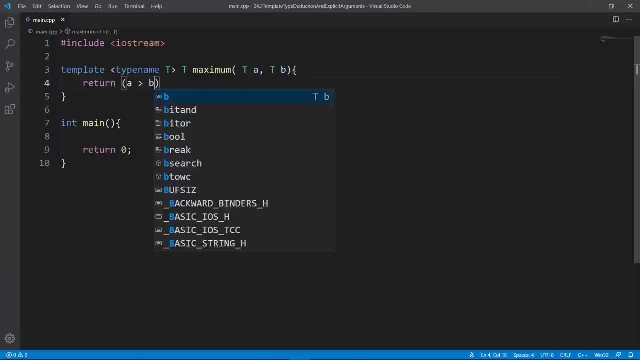 parameter is the maximum. we're going to say a greater than b: here we're going to use our ternary operator and we're going to say a greater than b- here we're going to use our ternary operator and if you want, you are going to click on your️ בה. CLICK here to go to the function templateINGS Gördnider over here, and you can. 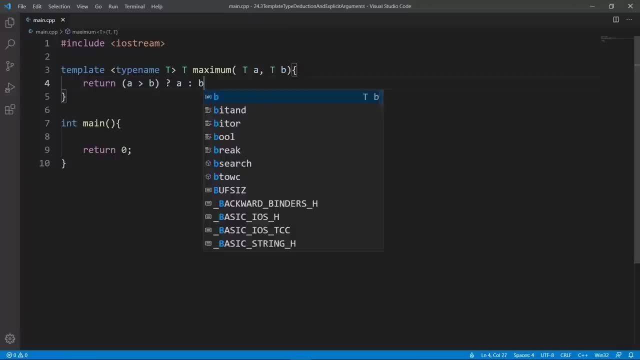 a is greater, we're going to return a. if b is greater, we're going to return b, and this is our function here. okay, now that this function is set up, let's set up a few variables to really play with that. so we're going to include the string library because we're going to be using it. a. 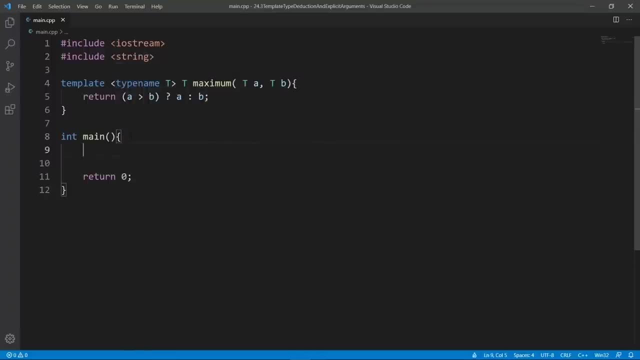 little bit and we're going to go down in the main function and put in our few variables. we have a through f here a and b are int, c and d are of type double and e and f are of type std strand. the first thing we can do, we can say auto max and we can assign whichever is the maximum between a. 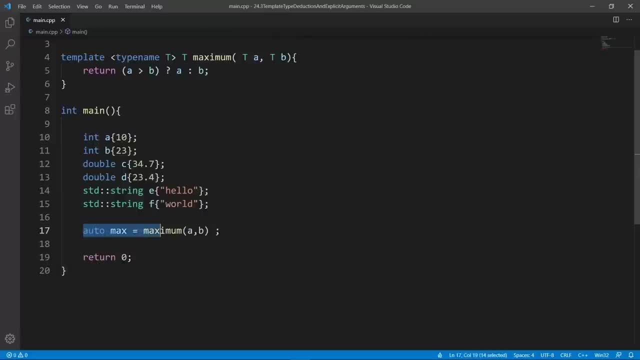 and b and once we do this we're going to have that maximum stored in max here. but what i want you to see is what the compiler does when it sees the call like this. the compiler has no other outside head to know the function template instance it should really generate. it is going to. 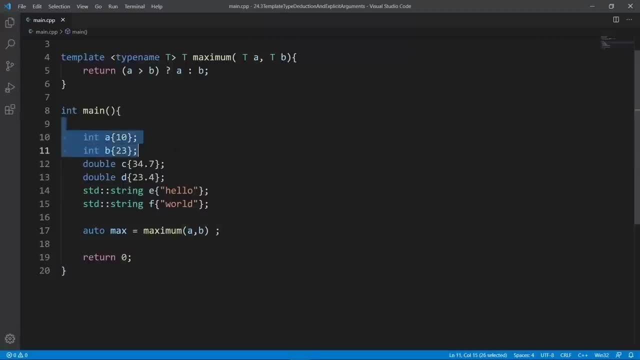 look at the types we have here- a and B- it's going to see that they are of type and it's going to see that it can use the function template we have here and it's going to use that and generate a template instance that it's going to. 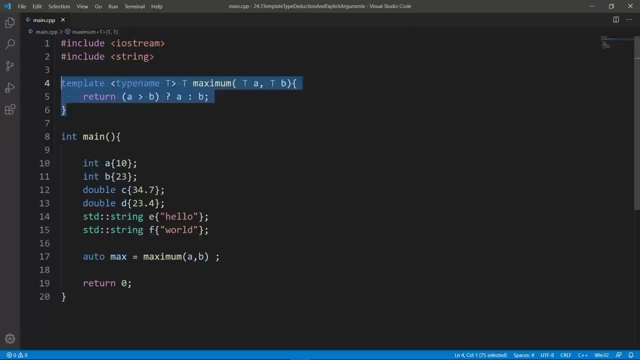 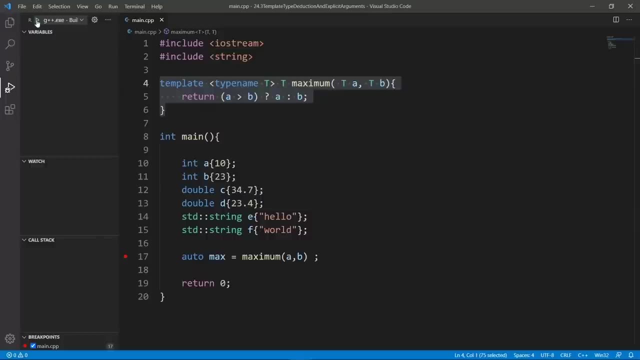 take and- and it is going to call it- to get our maximum here again. we can prove this through the debugger. we're going to set up a breakpoint, we're going to go to our run tab here and we're going to run this through our debugger. we're going to 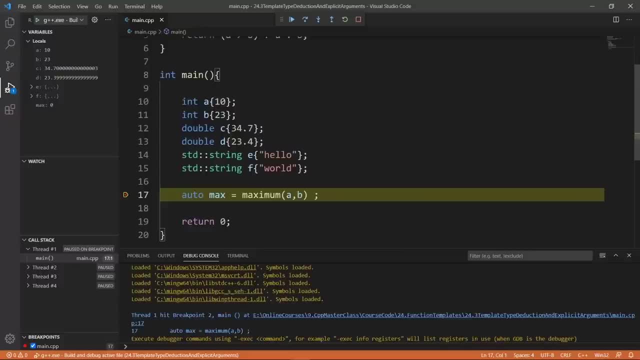 build our thing and when we hit the main function, you're going to see that a is 10, B is 23, which is what we have here. CD, we have our values, n and a steady strength, because it is a compound type or a custom type. we can expand on this. 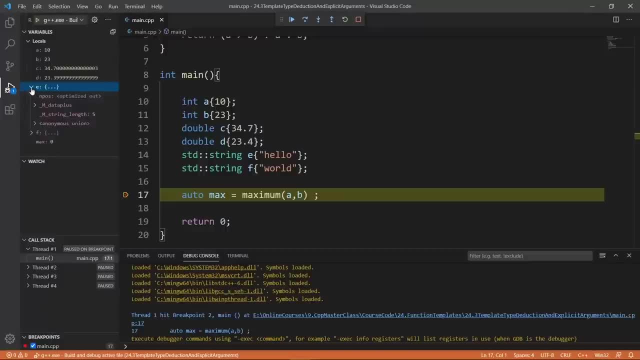 and really see more information about this, but we don't have enough tools to really understand this by now. so we're going to just to use this example here and we're going to run this through our debugger. we're going to as a wrapper on our string information here. now we want to call the maximum. 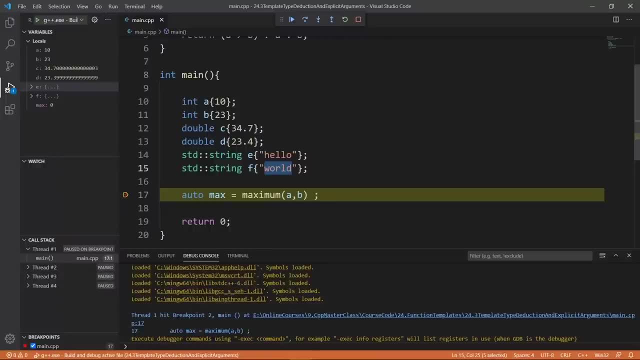 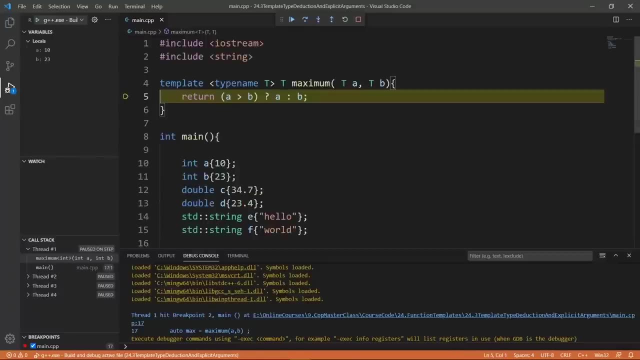 function and see what was generated by the compiler. and we can step into this function because we have hit the breakpoint by now. so if we hit step into, we're going to step into this function and we're going to see that it is an int function instance that was generated. this is enough for our purposes. if we 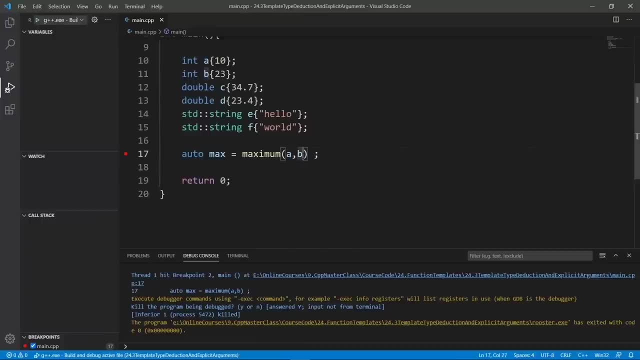 change our call here to use C and D, we're going to generate a double instance, so let's do that. we're going to generate a double instance and if we print this out, we're going to see this printed out. but we can use the debugger to really prove this. not that we know how to use it. we don't have to look. 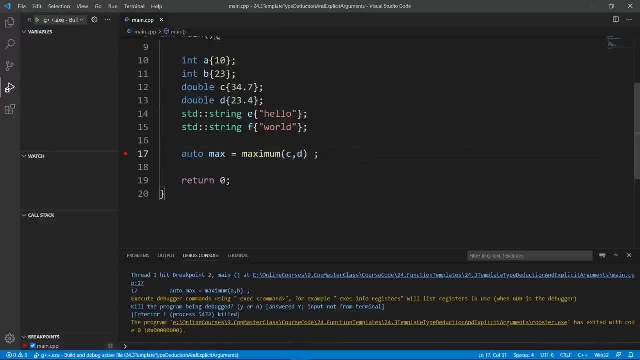 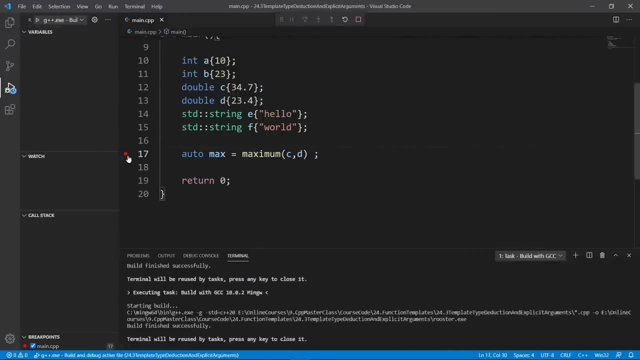 through the terminal output window. but you can do that if you want. you can set up STDC out and print max here. you're going to see it printed out, so let's run our debugger. we're going to see the template instance that was generated through the debugger. we're going to hit the breakpoint at line 17 here if we 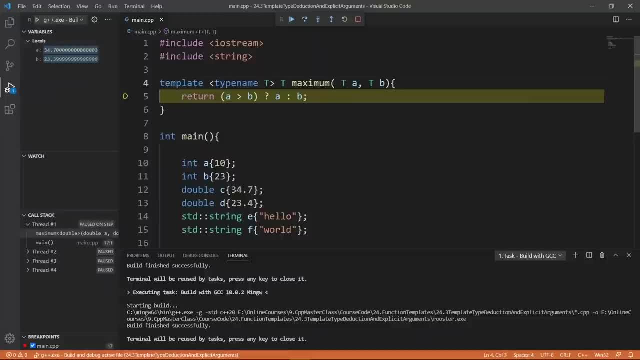 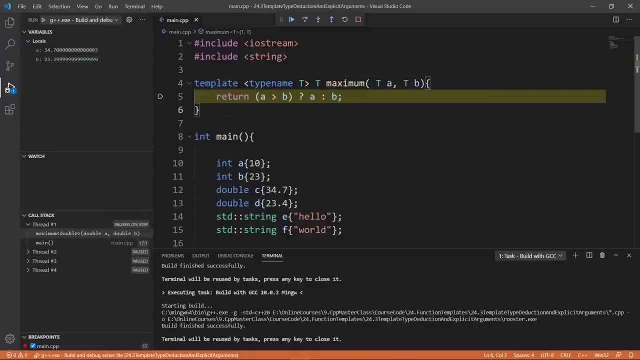 if we step inside, we're going to see the local variables for our function here, a and b- and we're going to have the maximum function to the top of the call stack and you're going to see that it is a double instance for our function. template here. okay, this is what we mean by template type. 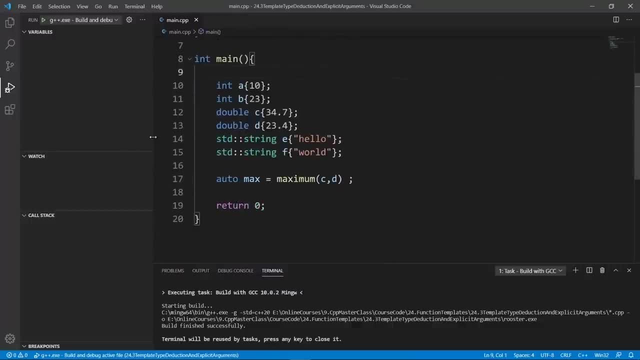 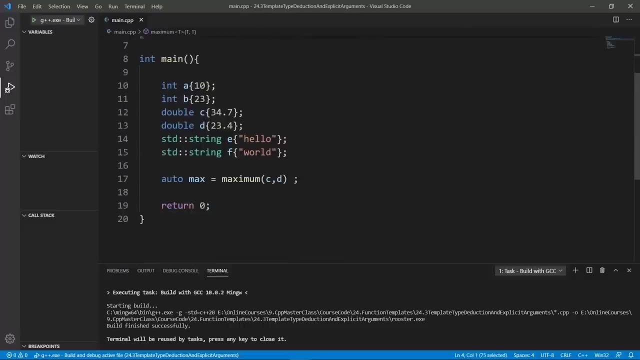 deduction. it is the default mechanism that the compiler uses to know which template instance to generate from your function calls. but, as we have seen in the last lecture, this can be problematic. one way this can be bad is if you pass different types to the maximum function here. 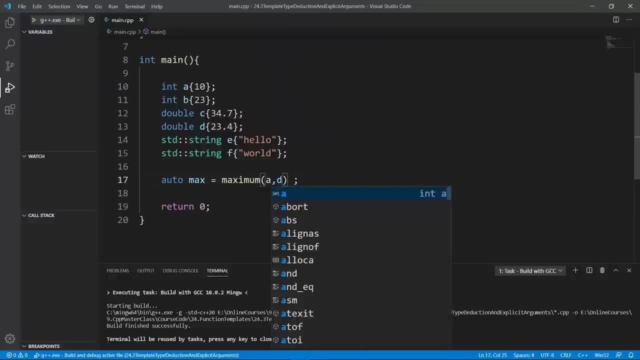 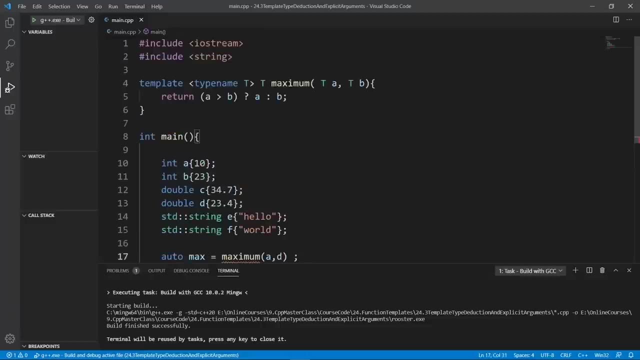 let's pass an a and c, for example, or a and d. this is going to work equally well. you see that we get a compiler error because the compiler now it sees that we are calling with different types, but the template parameters here are really of the same type. they should. 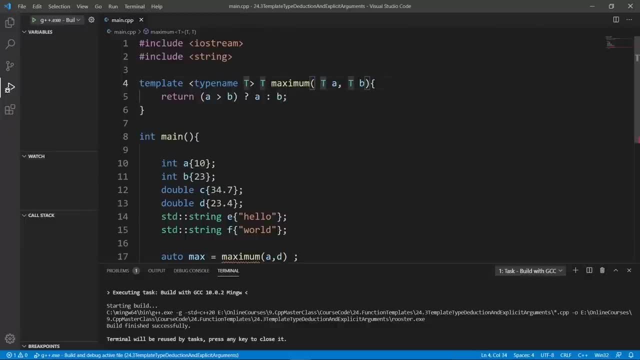 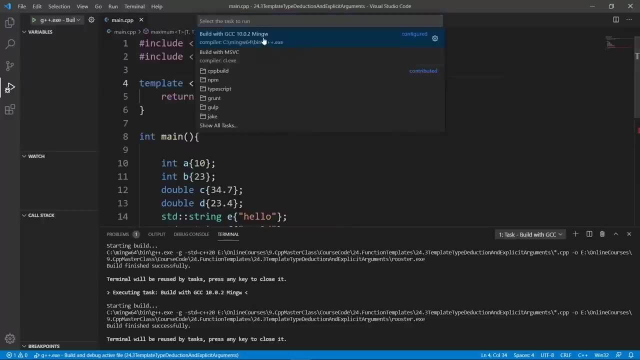 be of the same type, because t is going to be replaced for a single type. so the call we do here is going to fail. and if we run this through the compiler again, let's do that. we're going to use gcc. we're going to get a compiler error and it is going to say: deduce conflicting types for. 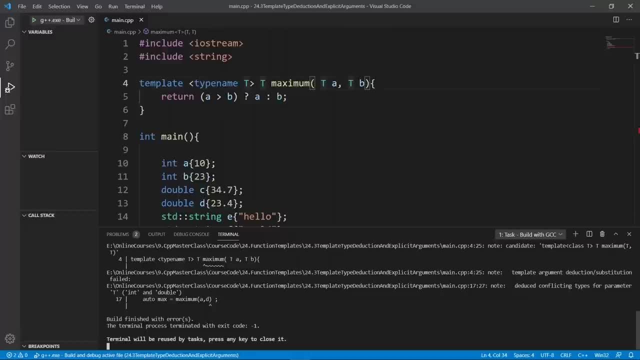 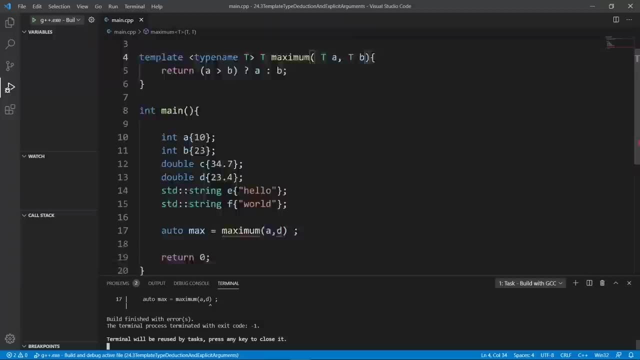 parameter t and double, so it can't really know which one you want. you want ant or double. the compiler doesn't know and it is going to give us a compiler error. but now we're going to see a mechanism we can use to make this work and that's going to be explicit template arguments. okay, what we can do to do this, we can. 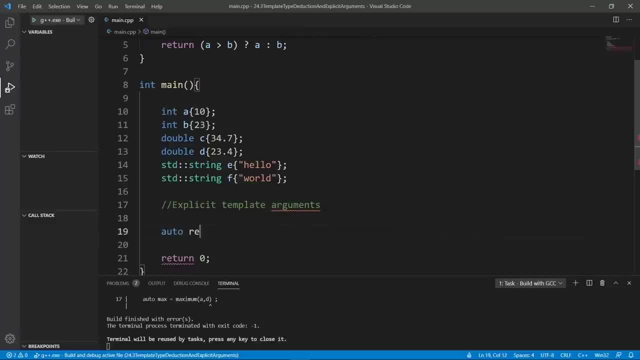 go down and put in our call. we're going to say auto and say result or max- we can call this however we want. we're going to save the name of the function and we're going to specify the template type that we want generated for our function template here. so if we do something like 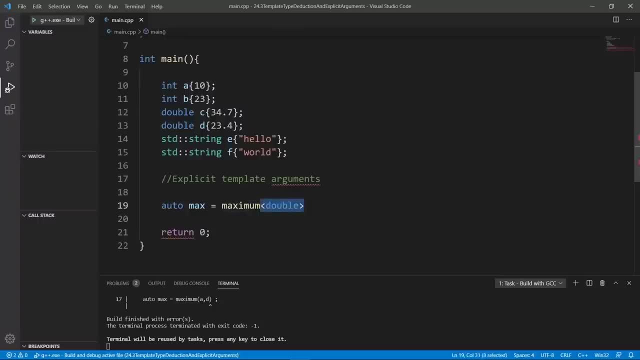 this with double inside angle brackets. here we're going to be basically telling the compiler: please generate a double template instance for this call we are doing here. so if we pass in c and d, for example, this is going to give us what we want and we can print this out if we want. so let's. 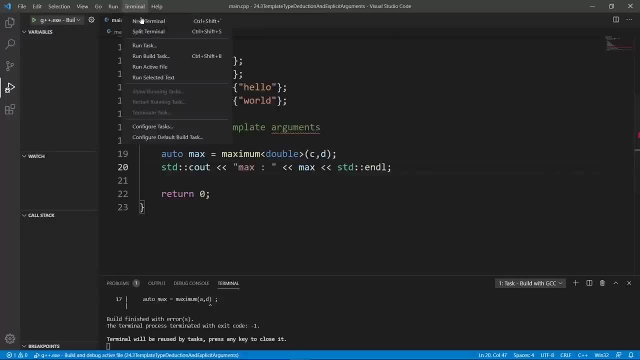 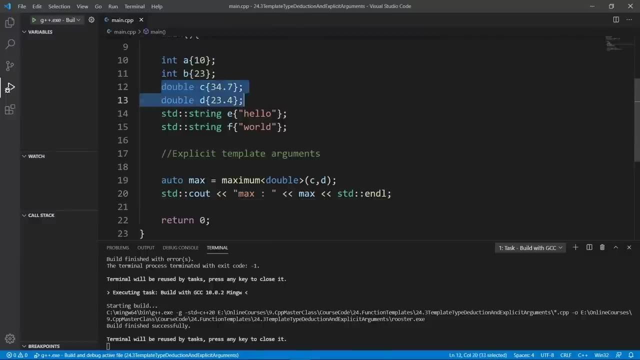 say max. okay, this is going to work. if we build, let's build with gcc, let's use that. the build is going to be good because we are passing any double arguments and if we run this, we should see our maximum. let's bring up a terminal window. 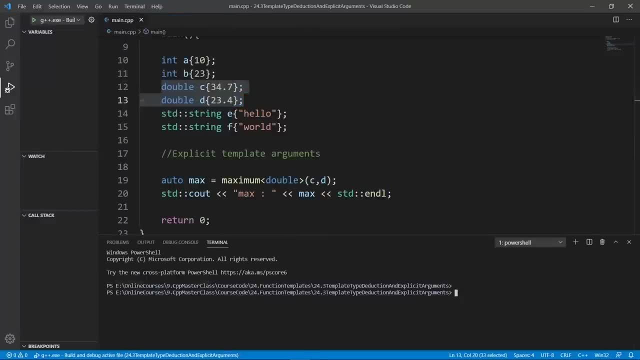 and visual studio code here so that we can use that to see things running. we're going to clear and run rooster. you see that we have our maximum here, but using explicit template arguments, like we are doing here, is going to allow us to even pass different types for our template arguments. 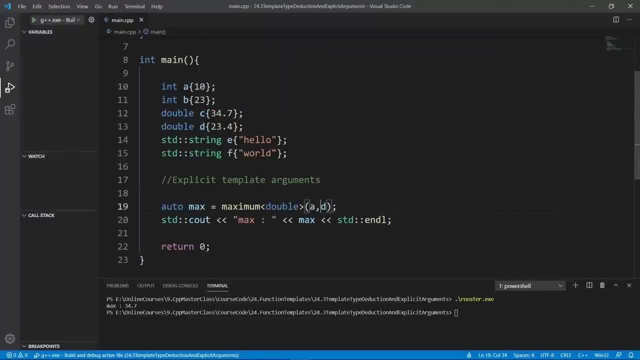 and, for example, now we can change the first argument here to b a, which is going to be an end, and we're going to leave the second one to bd, which is of type double. now the compiler is going to see that we're going to generate a template instance of type double. 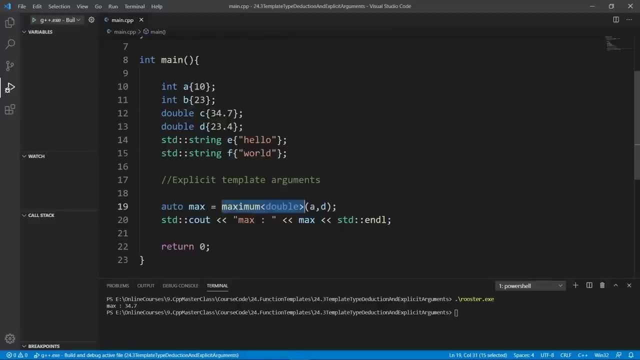 and it is going to know that it can do implicit conversions for the arguments we pass in here. so this is going to work if we pass an argument that is implicitly convertible to the type we passed in the angle brackets here. and let's debug this again to show you that. 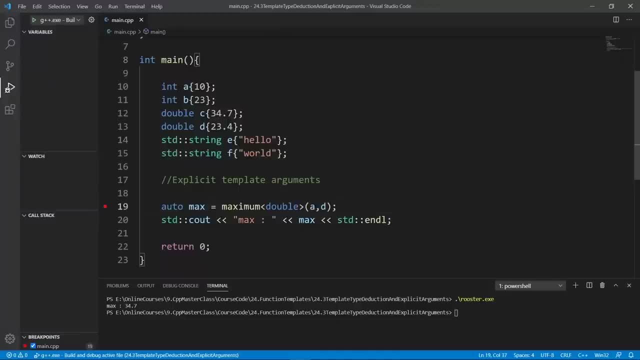 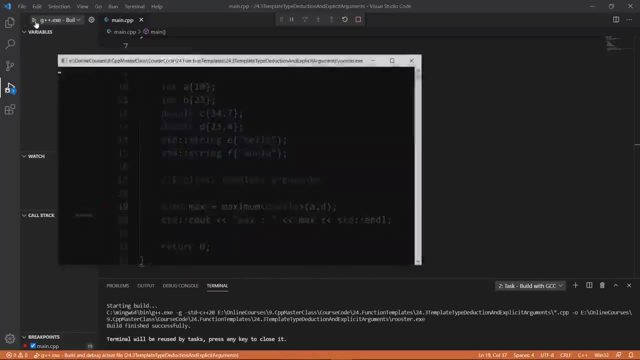 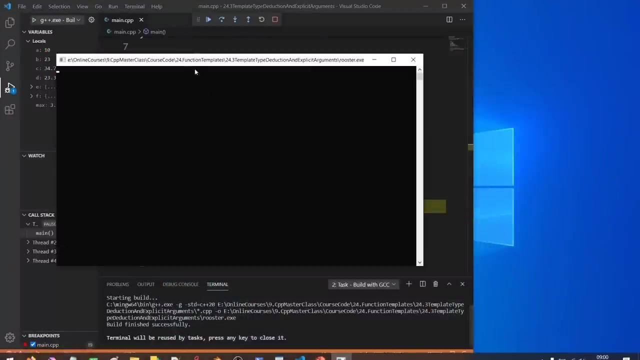 we're going to generate a double template instance that is going to be called and give us the maximum that we print here so we can run our debugger by hitting the green run button here. let's minimize this so that we can see our terminal window and it is down here. let's grab it and put it. 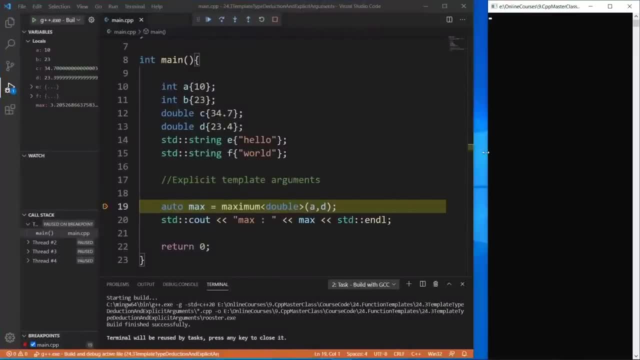 to the left so that we can really see things printed out as we debug. we have hit the break point here and we have our local variables. you can look at this if you want. it is basically what we have in the main function here, but what we want is to step into this maximum. 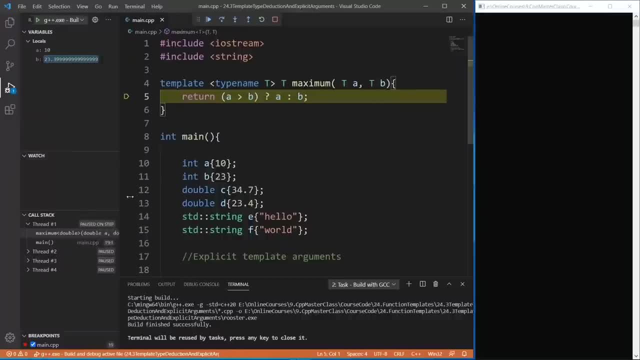 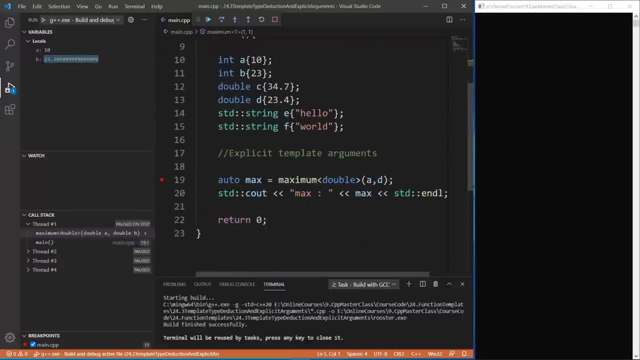 function and we're going to see the template instance that was generated. you see that it is of double type here. okay, hopefully now you can see that even if we passed different values for our template arguments, i should say different types, because a is of type and and d is of type. 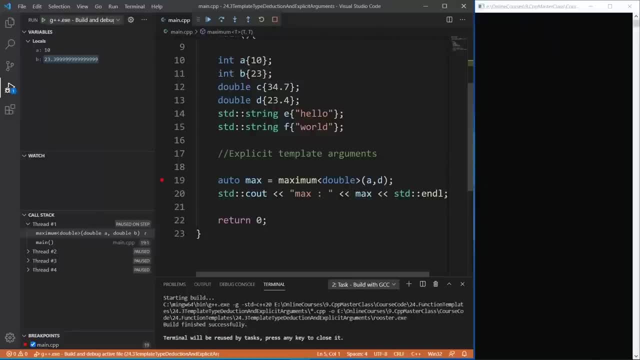 double, but we're not getting a compiler error. the compiler is going to insert implicit conversions from whatever arguments we passed here to the explicit template argument that we specified here. again, the explicit template argument, like we are doing here using the syntax with angle brackets and putting in our type, is: 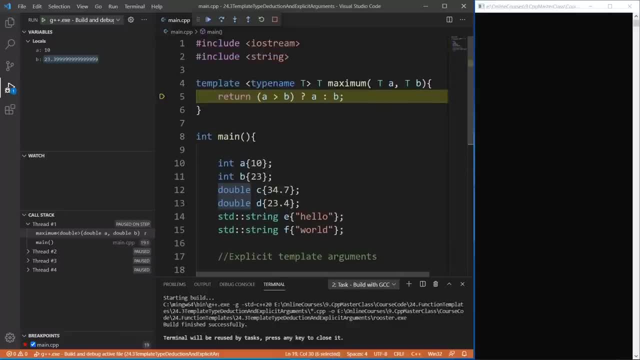 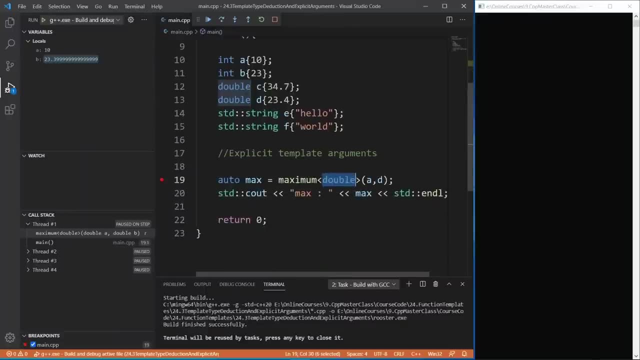 going to tell the compiler: please use this type and replace that for t in our function template here and generate a template instance. we can call to service this call here and we're going to do implicit conversions basically from end to double, because we're going to use this call here and we're 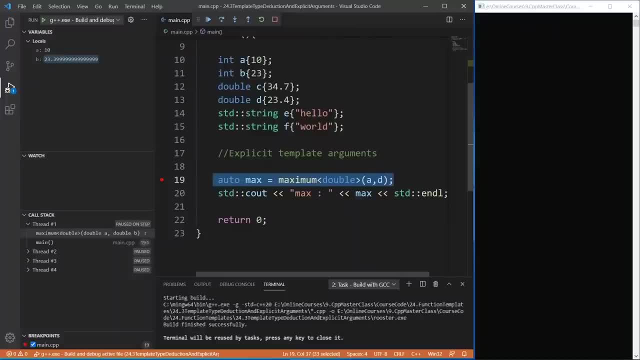 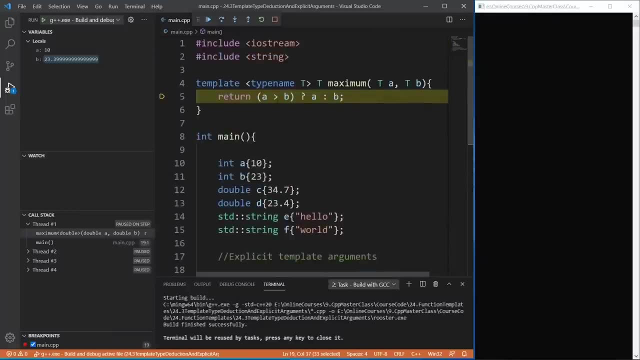 going to call this function because that's what we want, then d is going to be of double type. we're not going to do any implicit conversion. then we're going to call this function. we're going to return a double from it because that's our template instance and we're going to print that out here. 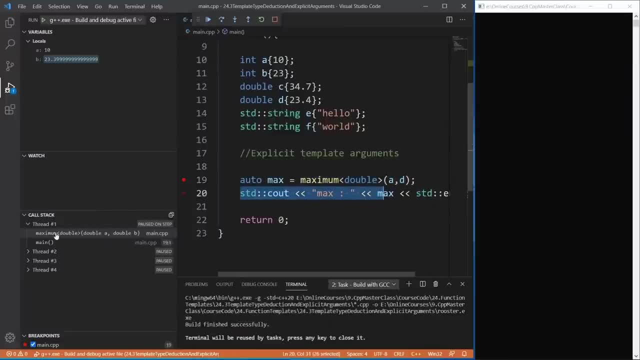 this is what is happening and we can prove that a double instance was generated through our call stat. here we see the maximum function is taking in double parameters and it's going to return double as our explicit template argument here. this is the syntax that gcc uses is using, but we know now that it is a double template instance. 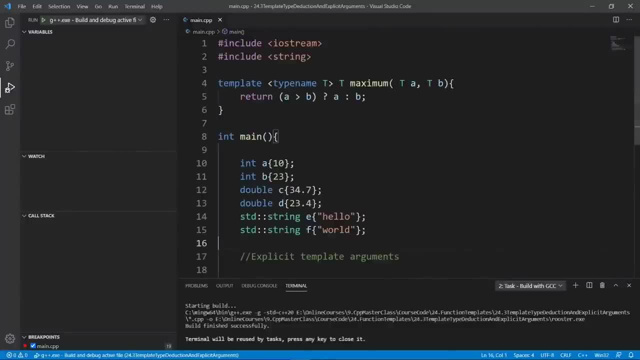 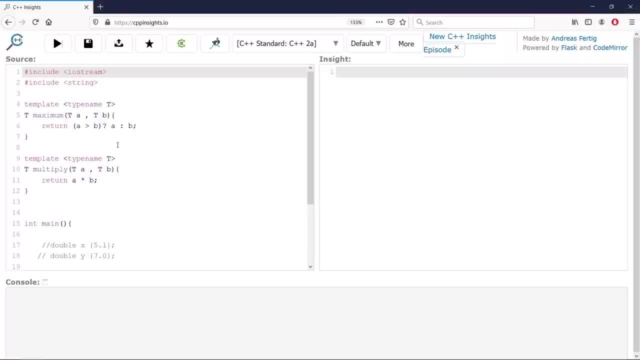 for our function. call here. okay, if you're not happy with what we are seeing with the debugger, you can also use cpp insights to really prove this. let's open this up. we're going to say cpp insights, let's do that and we're going to have it open here. okay, we're going to erase whatever we had. 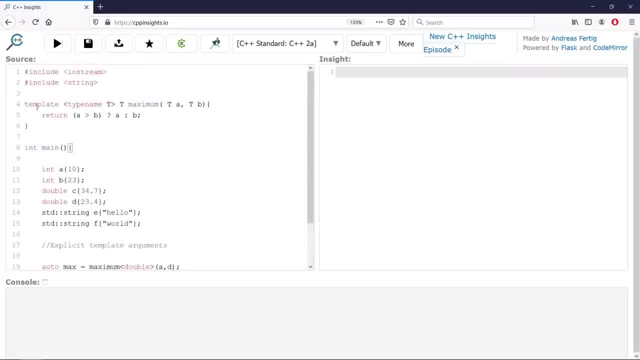 in here and we're going to put in another div function. now in the sais of code we have our maximum function- i should say template function or function template, and we have our call here and it is passing different types, a and d. remember the last time we did something like this by passing again different types for the template argument. 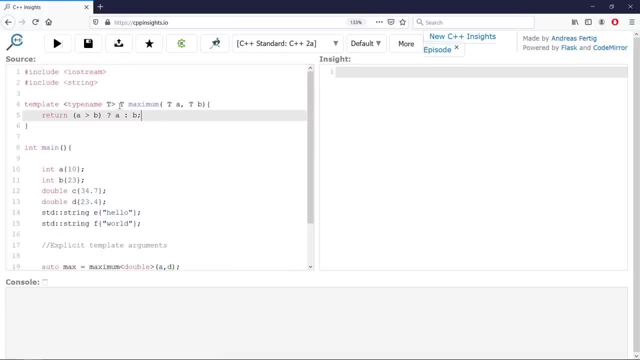 this guy failed. it couldn't really generate a function template instance because the template parameters we have on top here specify that these guys should be of the same type, able to use different types as arguments, because we have an explicit argument specified. let's run this and see the template instance that is generated and you can see that it is of double. 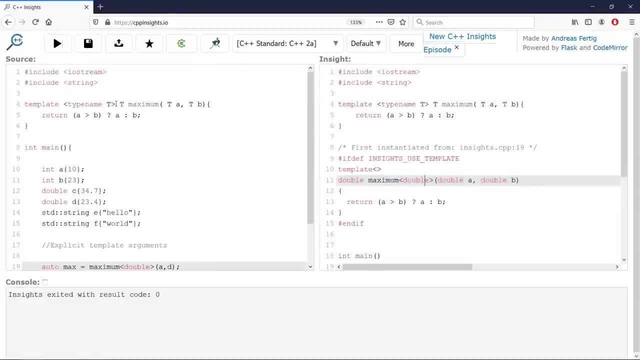 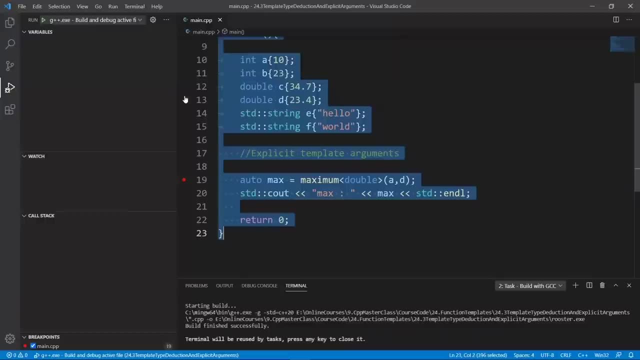 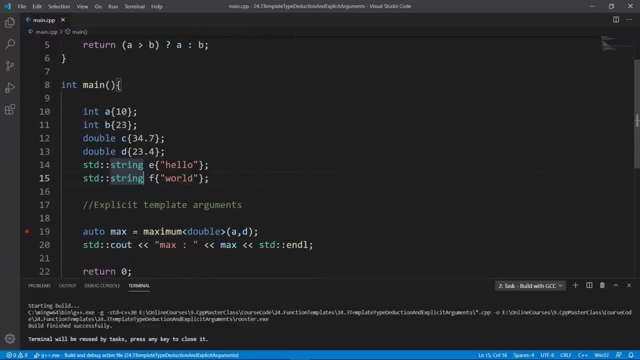 type. we basically replaced every instance of t here with double and this function is going to be called to surface, the call we are making here. okay, this is really all we set out to do in this lecture. i hope you found it interesting. the main message was template type deduction: a default. 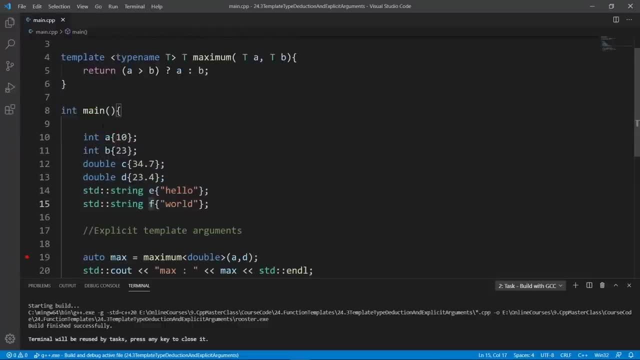 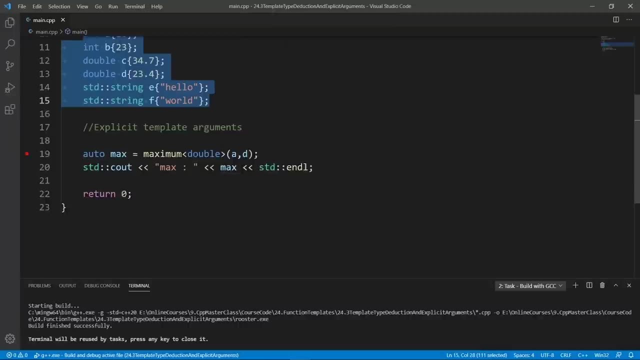 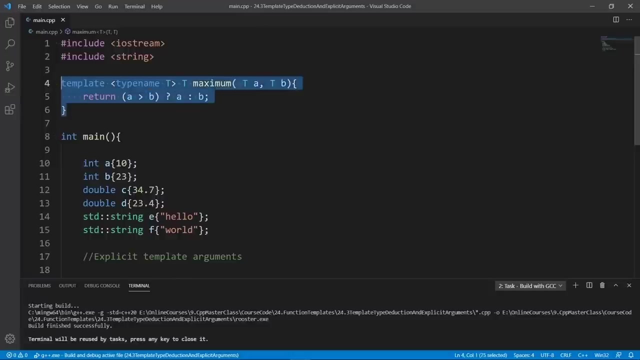 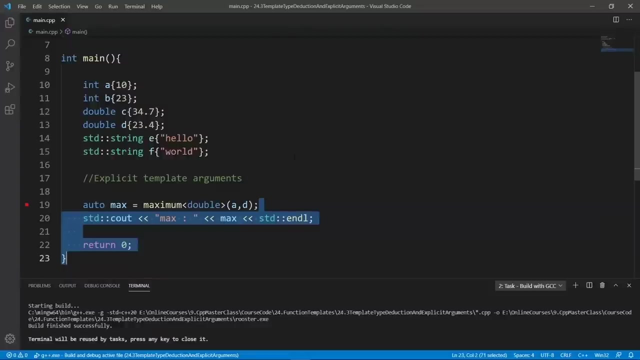 mechanism c plus plus uses to know which template instances to generate from your function calls. but if the defaults aren't working for you, you can use explicit template arguments to specify the template instance you want generated. we are going to stop here in this lecture. in the next one we're going to see how we can pass template parameters by reference. 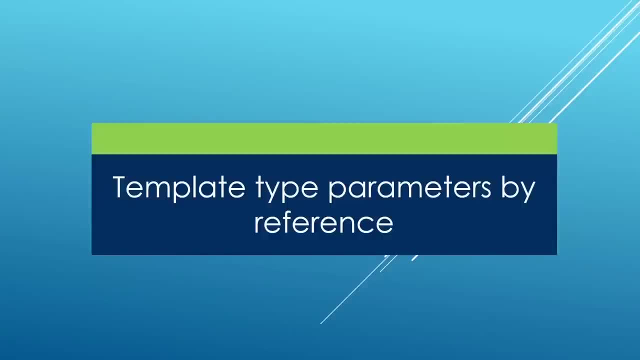 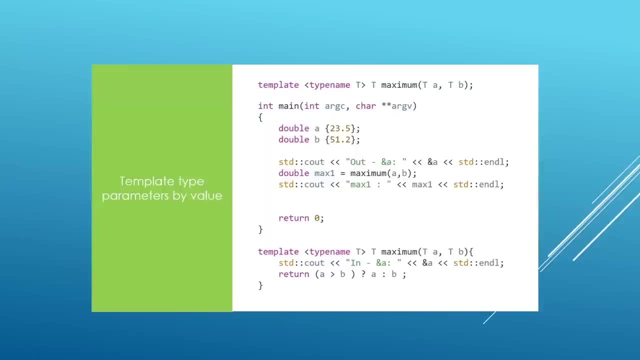 after we're done, we're going to look at other instances. go ahead and finish up here and meet me there. in this lecture, we're going to show you that you can pass your template type parameters by reference and we're going to look at a simple example to really drive this home: what we have. 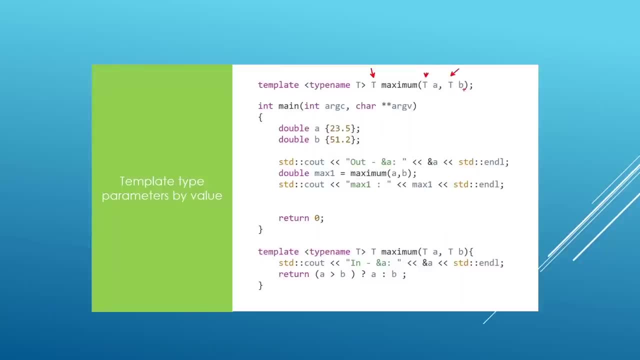 said so far is that we can do things like this and specify our t like this, and this is going to generate a template instance that passes arguments by value. for example, if we pass in double a and double b here for our maximum, a template instance which takes double as parameters and returns the double here and 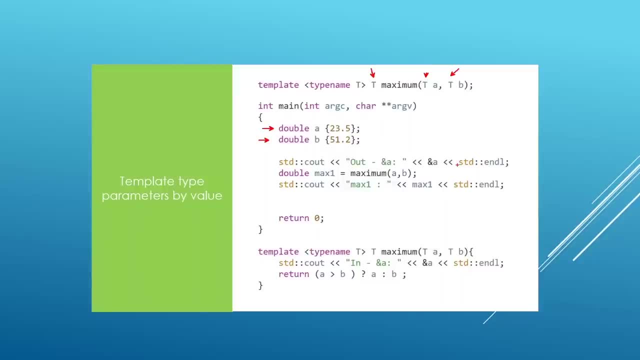 this is going to be doing things by value. okay, this is what i want you to focus on right now. it is that this is going to do things by value. so if we go in our function here and compute the maximum, you're going to see that the addresses we have on the outside are going to be different from 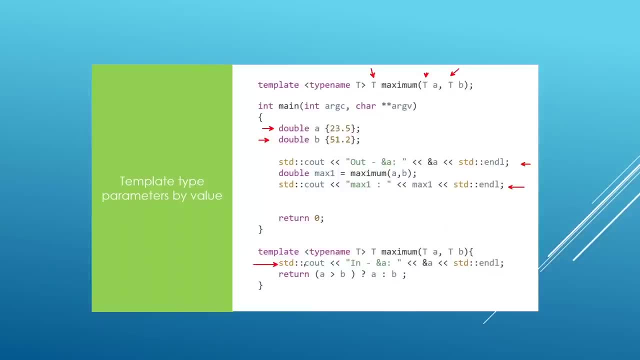 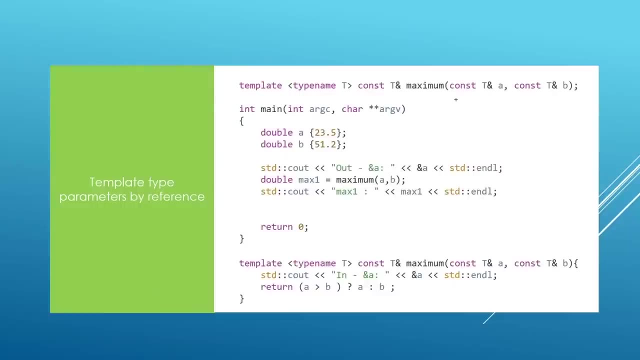 the addresses we have on the inside here if we're trying to print them out. but you can also pass your template parameters by reference and the syntax to do that is ridiculously easy. you just use this like you would use any reference. we say cost t reference here and this is going. 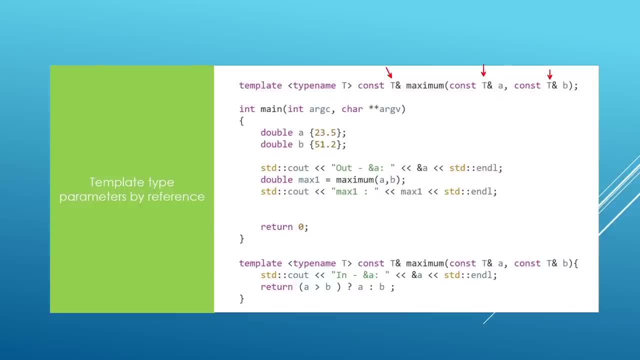 to just replace in whatever type that you pass when you call the function here. for example, here we are passing in double arguments, so this is going to deduce a double template instance which basically says cost double reference maximum, cost double reference a and cost double reference b, and this is going to be the function that is called. so this is going to really do. 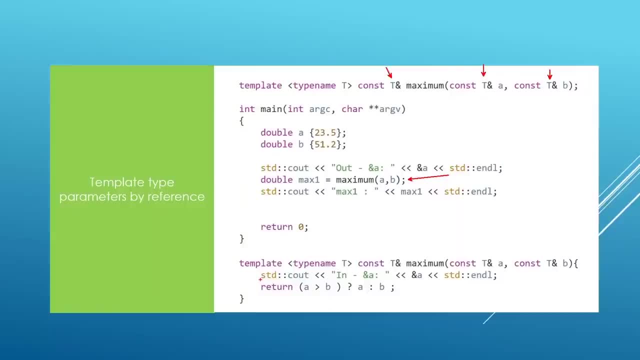 things by reference and the values we have inside our function template body here are going to be true references to the values we have on the outside. if we happen to do any modification inside the body of the function, the modification is going to be visible on the outside. what we're 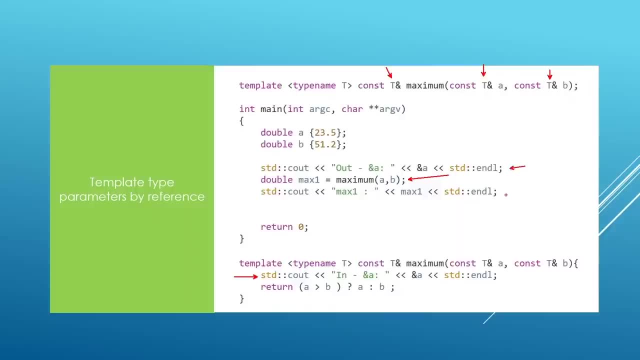 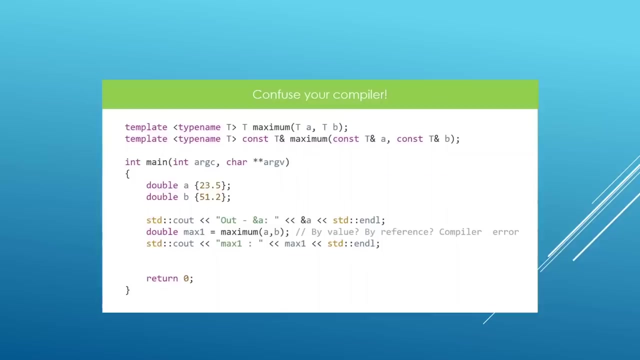 going to be doing in this lecture is just printing the addresses here and we're going to see that they are the same here on the outside and inside the body of our function template here. okay, this is what we want to really play with in this lecture. but before we head over to visual studio, 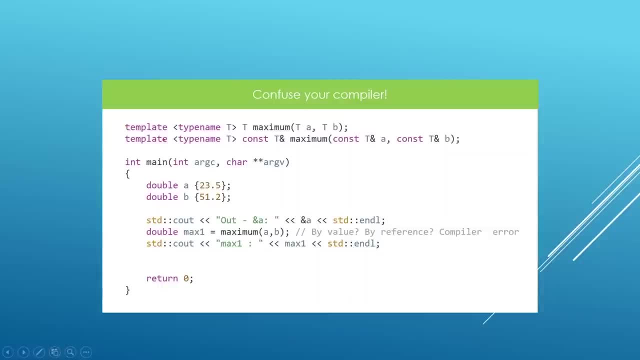 code. i want to show you that you can confuse your compiler if you are not careful. if you set up these two function templates you see here they are going to be overloads and we can use function overloads with templates. but for now we're just going to focus on the parameters that we are. 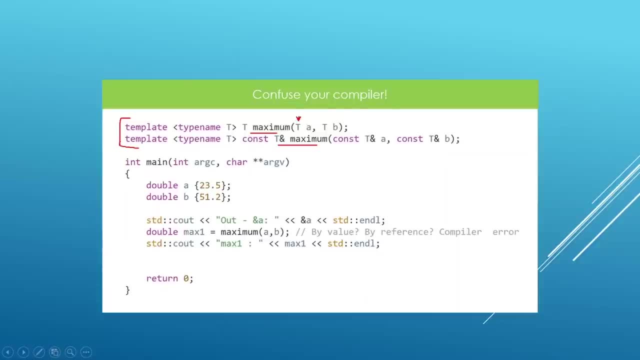 passing on to you, and we're just going to focus on the parameters that we are passing on to you in here. the first one is taking things by volume and the second one is taking things by reference, as we see here, and if we issue a call like this, we're going to have the same problem we have seen. 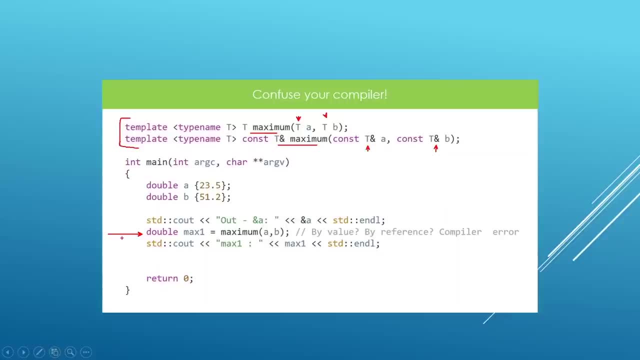 with function overloads before. this is not going to know whether you are calling by value or by reference, and this is going to cause a compiler error. i really want you to be aware of this. okay, now that you know this, we're going to head over to visual studio code and really play with us. 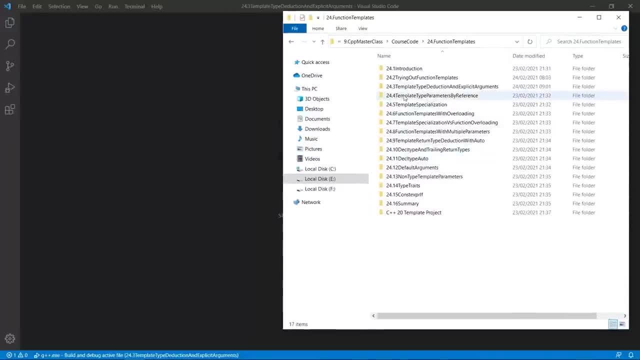 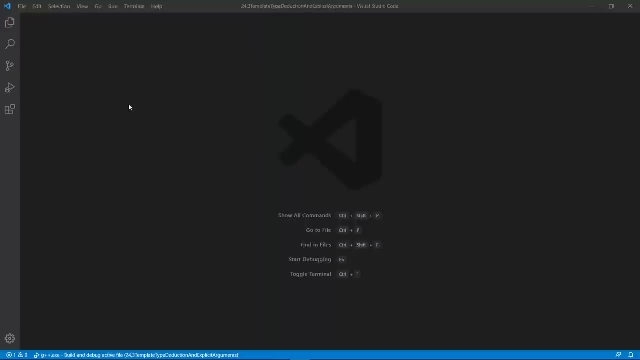 a little more. okay, here we are. we are in our working folder. the current project is template parameters by reference. we're going to grab our template files and put them in place, so let's do that, and we are going to open this little guy in visual studio code by dragging and dropping here. the folder is going to open. 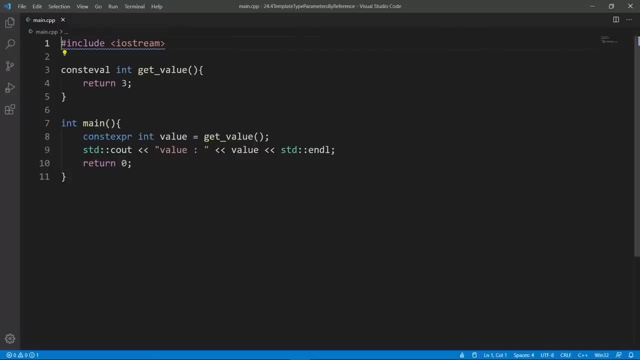 up, we're going to open it and we're going to close the left pane here and clean up our main file here and we are going to put in our function template. one thing i want you to see in this lecture is that it is possible to separate these things into function declaration and function. 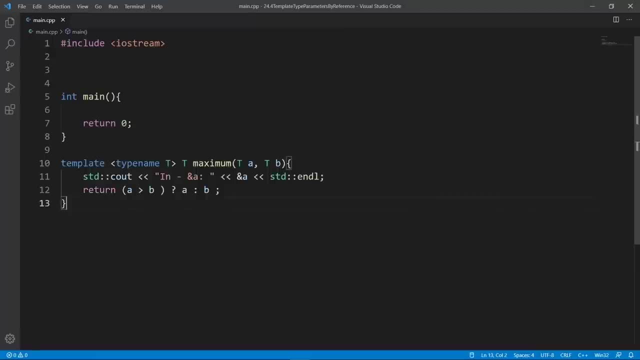 definition. let's just try and do that here so that you can really see this, and then you're going to have to choose what you like a little more. so let's grab our function header here and use that as our prototype. we're going to put that in front of the main function and that's going to be our. 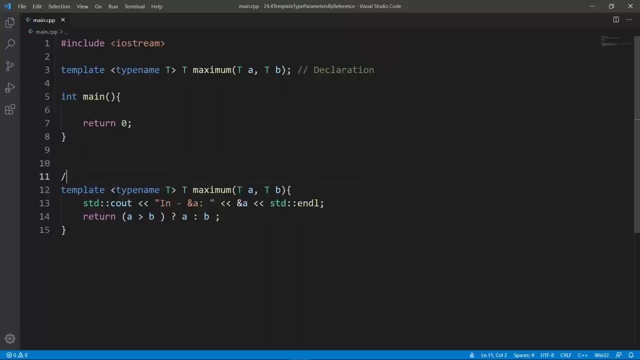 declaration and if we go down after the main function here, what we have is our definition. this could work and this is going to generate template instances for the calls we do in the main function here. okay, now that we have this, we can head in the main function and really play with the function template here we're going to set up. 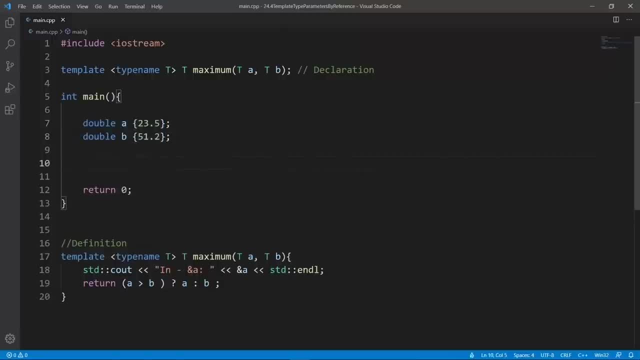 two double parameters and we're going to call the function. for example, we say auto result and we're going to call the maximum function and we're going to pass in a and b. this is going to do default template type deduction and it is going to generate a double function template instance here. 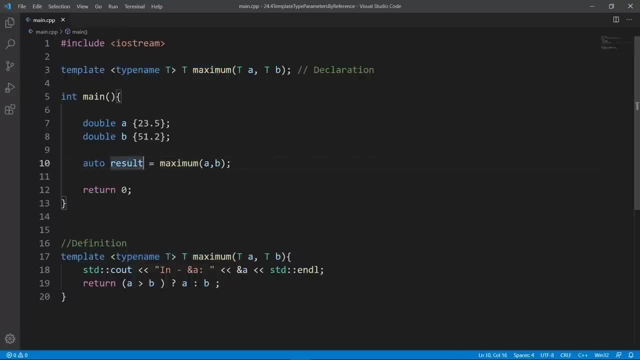 what we really want to prove is that this is going to pass things by value, and one way we have to prove this is to print the addresses both on the outside and on the inside of the function. here, you see, we are already doing that in our function template body. we are going to print the address of 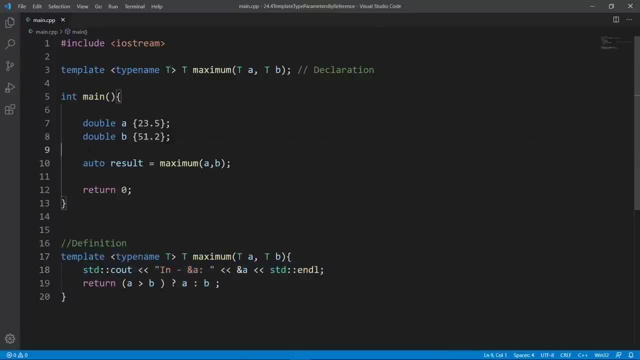 a. so we can really grab this and reuse this stdc out statement and we are going to change it to say out here and we're going to print the address of a. let's grab this again, use this after the function call and what we expect to see is some address on the outside. 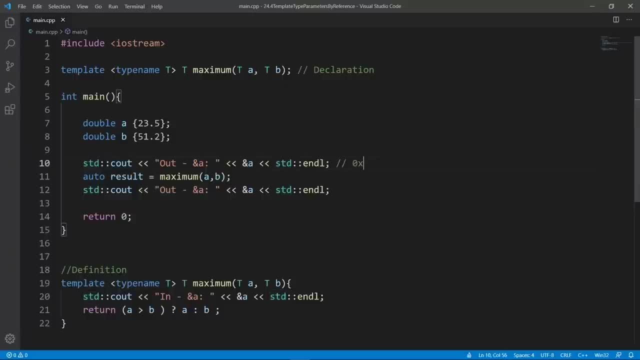 so, for example, we may have something like 0x and a, 1, 1, 1, a, b, c, which is some hex number here- and that's the same thing we're going to have on the outside, because the value we have before the function call and the value we have after the function call are going to be leaving at the same address. but what we have inside the function call is going to be leaving at the same address. but what we have inside the function call is going to be leaving at the same address. but what we have inside the function call is going to be leaving at the same address. but what we have inside the function. 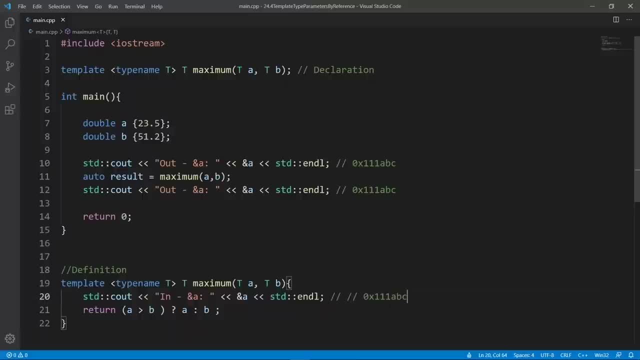 function body is going to be a copy, so it's going to live at some other address, for example, let's say d a, and the main point here is that what we have on the outside is going to be different from what we have on the east side, and hopefully this is going to prove that we are passing by value. 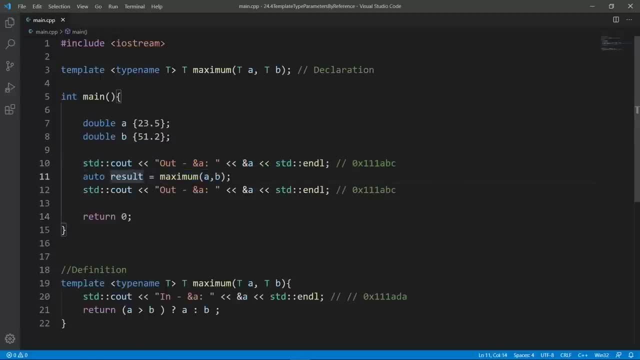 so let's print out our maximum here and see the addresses printed out. we're going to build with gcc and we're going to build successfully. we can bring up a terminal to play with us a little more and we can clear and run rooster. we're going to see that the address on the outside ends in dd8. 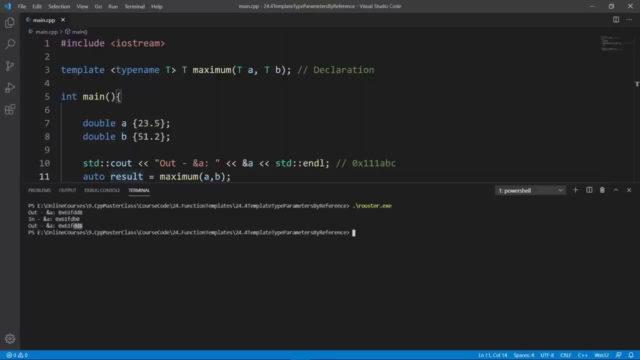 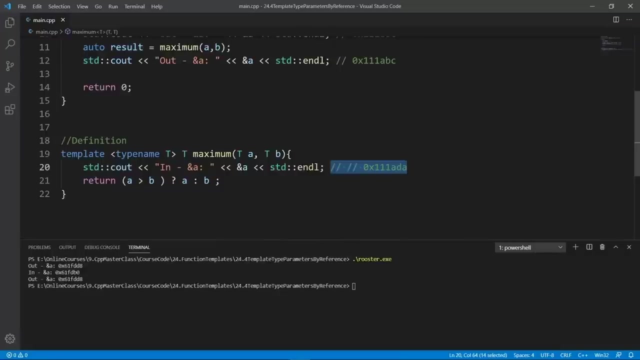 and the address on the outside ends with dd8 after the function call. but inside you see that we have a different address and this is going to tell us that we are passing by value and what we have inside the body of the function is basically a copy. again, i don't expect you to see the same. 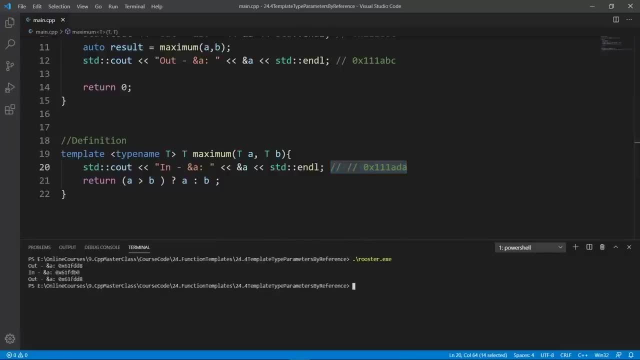 addresses as me here, because your operating system is going to set up the addresses however it wants. the main point here is that the addresses you see on the outside are going to be different from the addresses you see on the inside here, and this proves that we are passing by value. 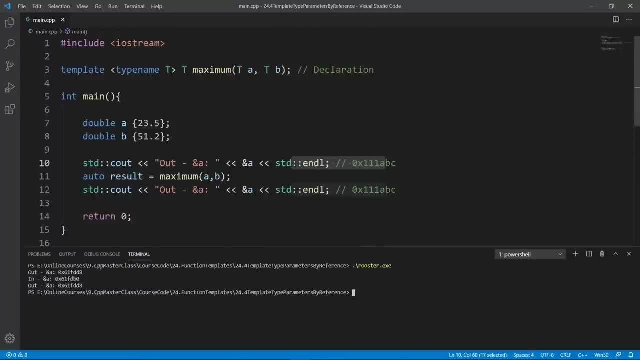 but what if you don't really want to pass by value and make your function template work by reference? well, we can do that. we can change our function here to do things by reference and all we have to do is use t reference like this: okay, and when we start using references, we really need 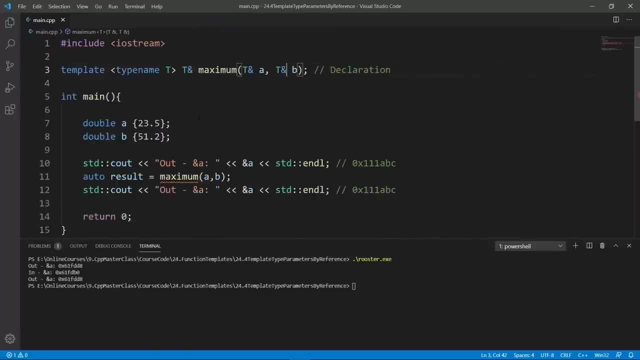 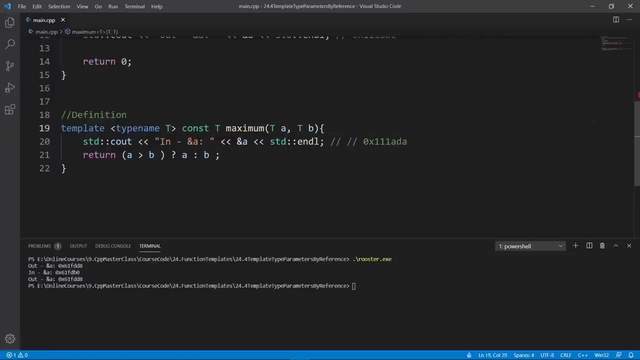 to be careful and make sure people don't modify things without our knowledge, and a good practice is to mark your things as cost references. so we're going to do that, and we are going to do the same in our function definition. so we're going to change this to cost t reference. let's do that. 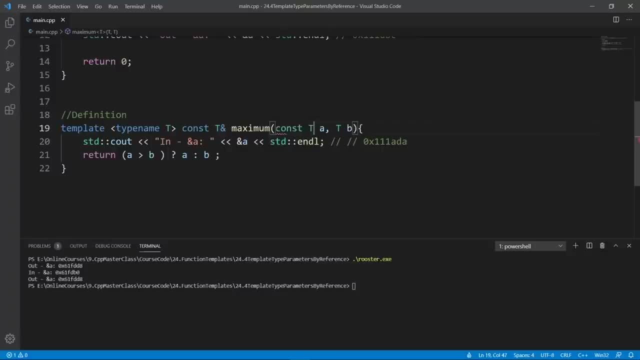 and then say cost t reference for the first parameter here and say the same for the second parameter here. and this should be it. we shouldn't be able to use this reference to modify the data inside the body of the function, and our function is a little surfer. 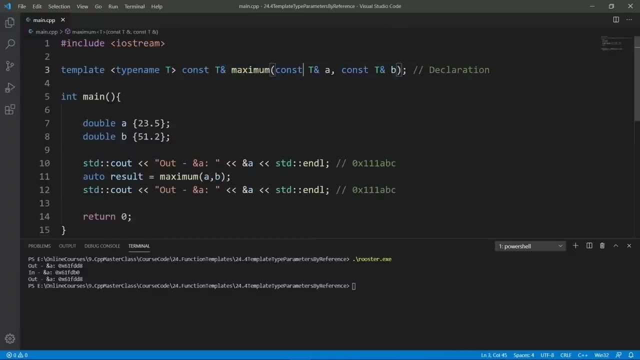 but what the compiler is going to do is really what it's been doing all along. it's going to look at the arguments that we passed to the function call here. it's going to see that it is double and it's going to do default template type deduction, so it's going to generate. 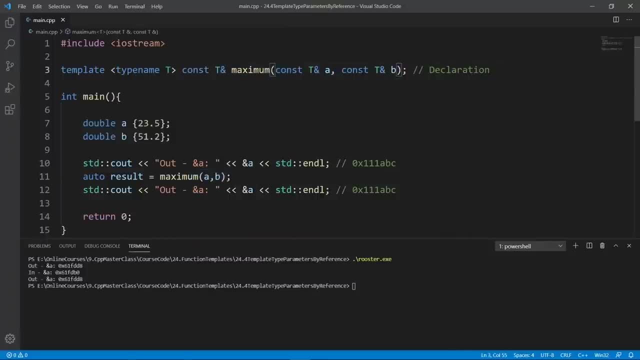 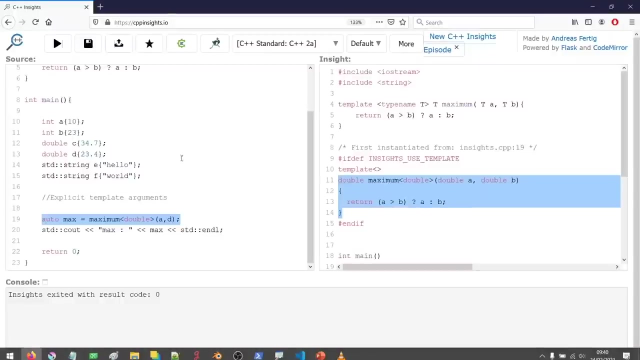 a double template instance for the function template here and it's going to replace in double and we're going to have const double reference, maximum cost double reference plus reference reference a, constant double reference b and we can prove this by going into cpp insights. i think we can do that. so we are here in cpp insights, we can take out whatever we had we're going to put. 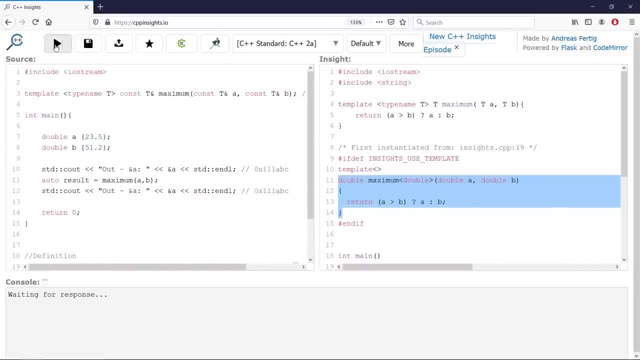 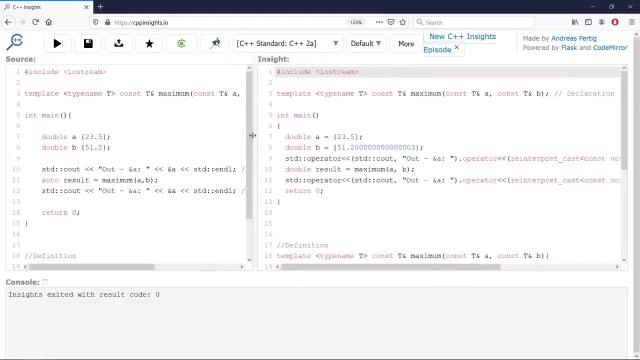 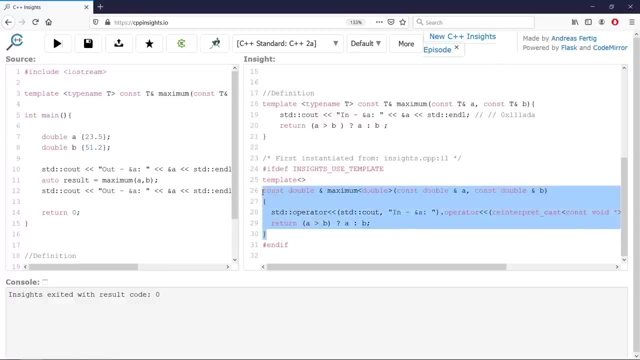 in new code here and we can hit the run button to generate our instances. and here we have our template instance here generated. you see that it is going to generate a double version of our function template here and this is what we have, so constant double reference maximum and it is. 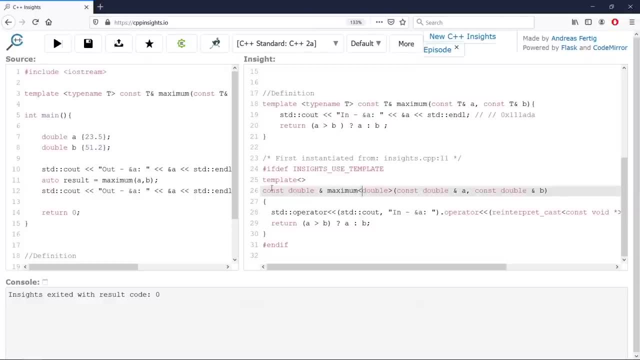 going to put in a double explicit argument here. but this is business of the compiler. what we really care about is that it generated a double template instance for our function template here. now, if we run this, it is going to be passing parameters by reference and what we have on the 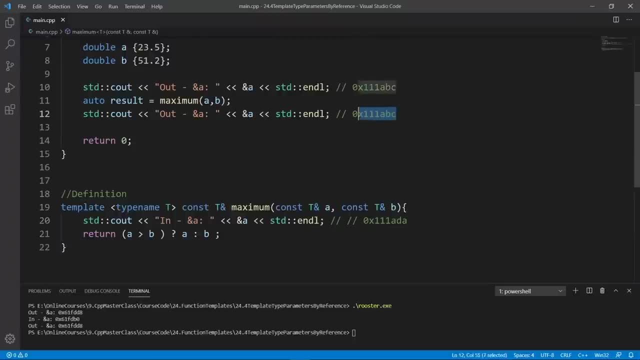 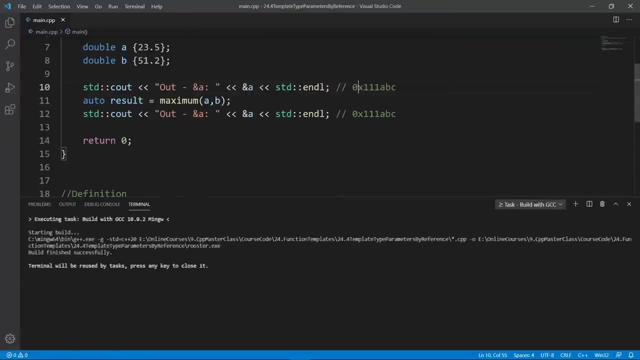 inside should have the same address as what we have on the outside here. so to really drive this home, we should change our address to abc to comply with what we have on the outside. here we can try and build our program. we're going to use gcc to do that. the build is going to be good. we're going to 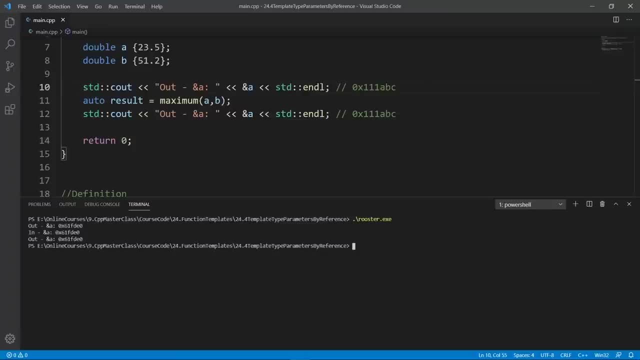 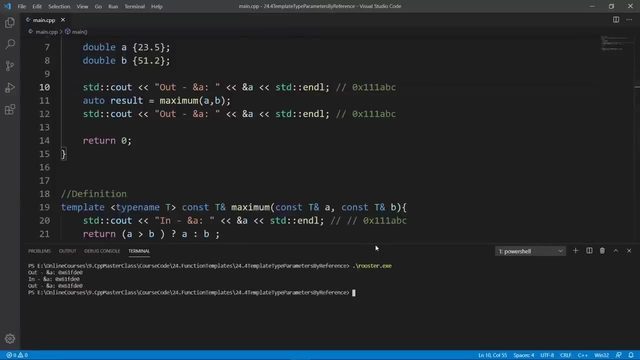 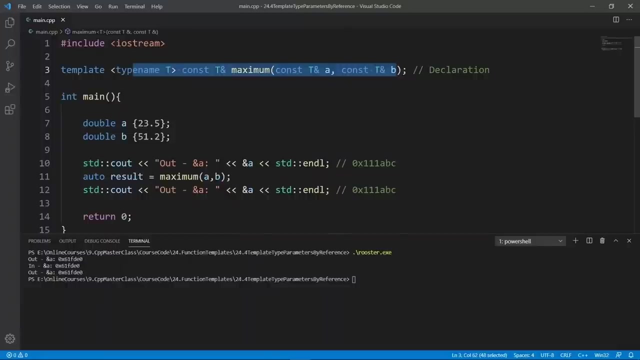 clear and if we run rooster, we should see the addresses being the same: out de0, in de0 and out de0. and you see, now we are passing our parameters by reference. and if you want to set up a function template that passes template parameters by reference, this is how you can do this and i think we can also try and debug this and see if we 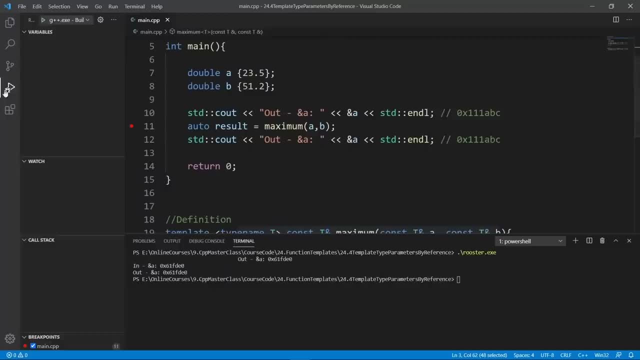 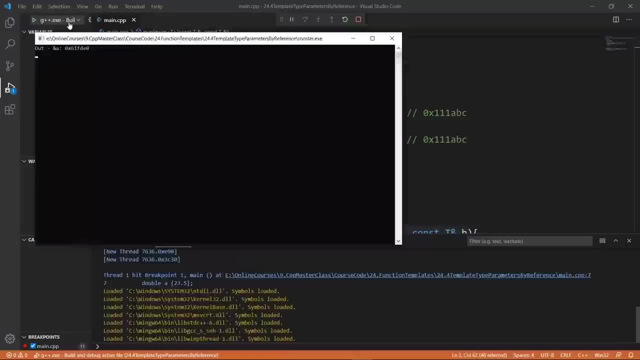 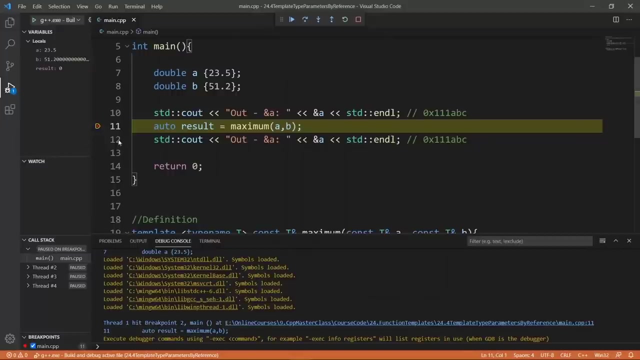 can see any more information on how this works. we're going to hit our run tab here and we're going to hit the green button to start debugging this program. we're going to be using the debugging tools from gcc and we see our local variables here. we have hit the breakpoint and we have the. 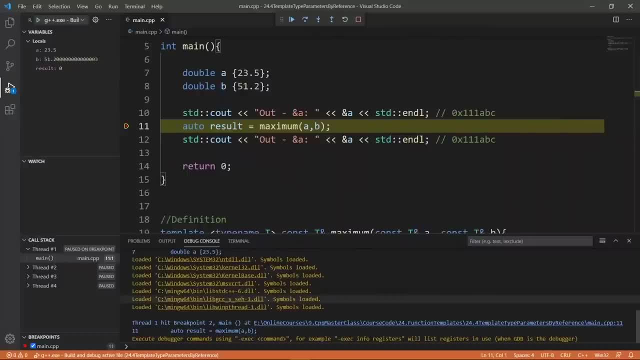 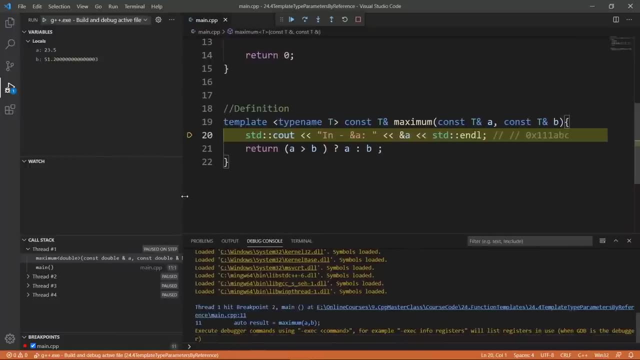 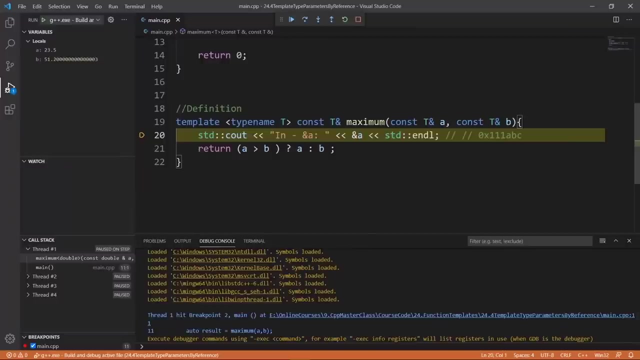 main function to the top of the call stack. this is what we see we have here, and if we try and step into the maximum function, we're going to see that the template instance now is using const double references and this is the template instance that was generated. i think this is all we can really see here, and let's stop this and show you. 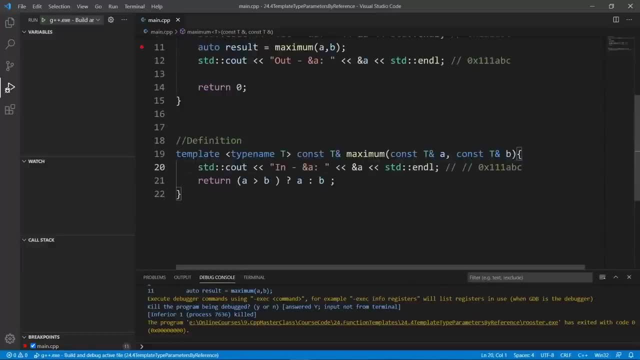 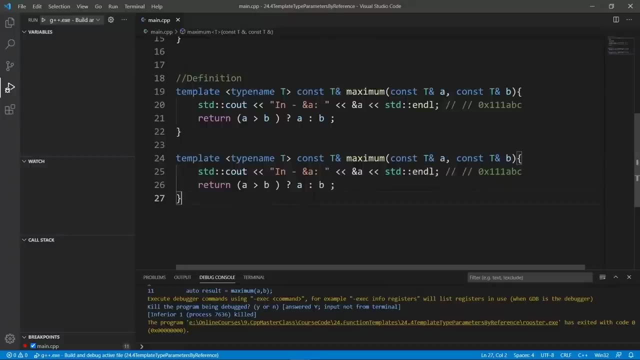 one last thing. what i'm going to show you is that you can't really have the function template that passes by a value and the other one by reference. if you do that, you're going to have problems when you issue the call like this, because the compiler is going to be confused. let's change the second one here to pass by value, so we're. 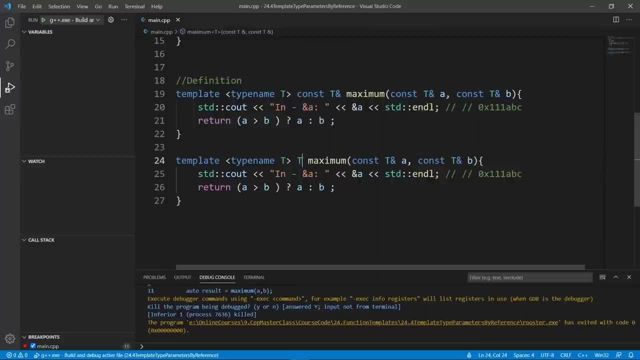 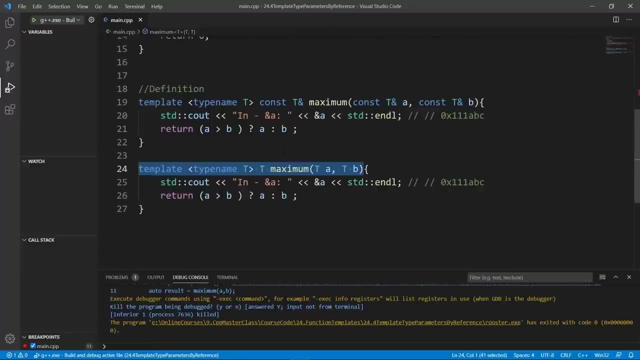 going to remove the cost reference here. i think it's going to do. let's do that pretty quick. we remove the cost and the reference. we remove the cost and the reference here and we use this guy as our function prototype in front of the main function here. and how can we say that we're going? 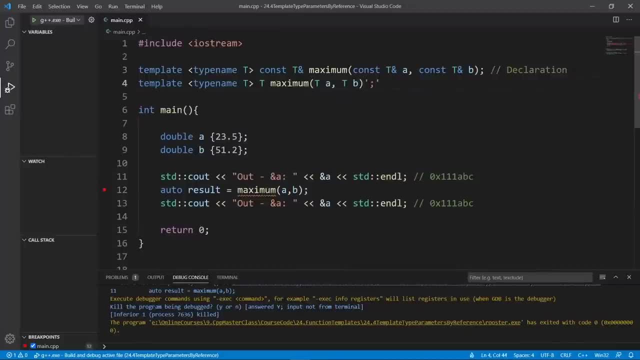 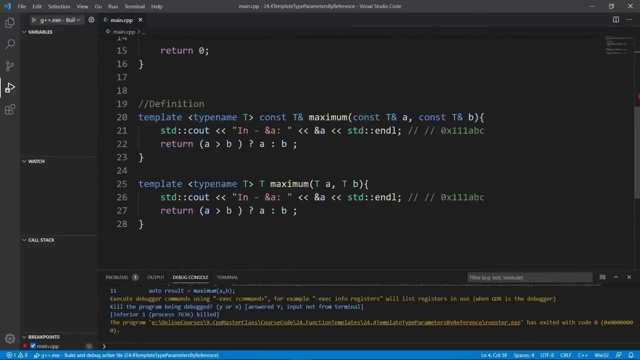 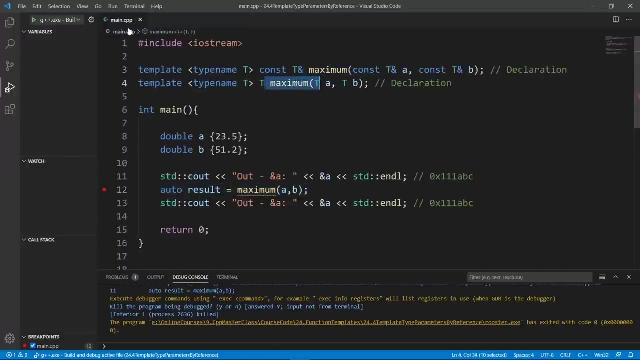 to go on top here and say that, okay, we're going to put our semicolon and this is going to be our declaration. but the moment we do this, you see that our compiler is going to be confused because we have two possible candidates for the call here. it can either be by value or by reference, and if we 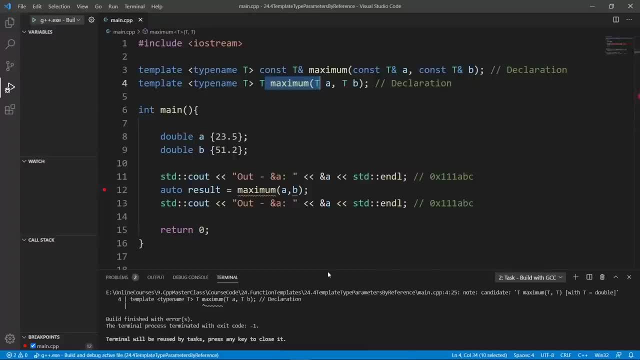 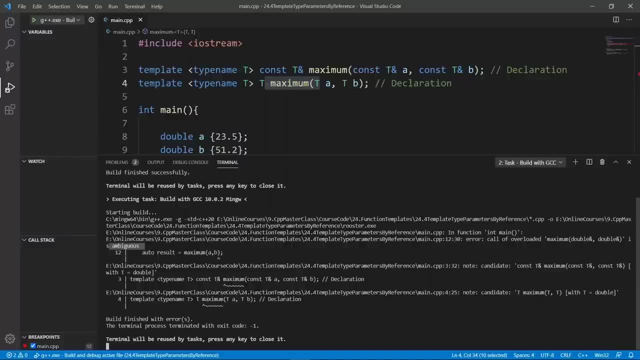 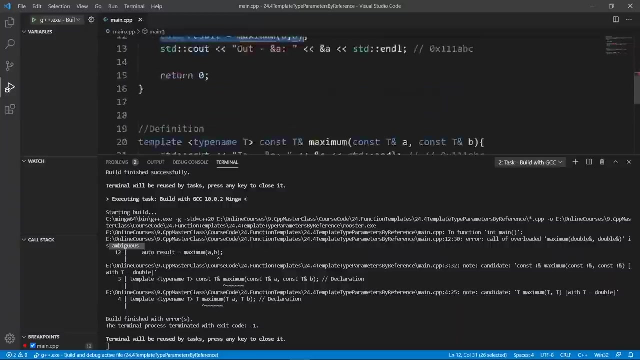 try to build this program, we're going to get a compiler error and it is basically going to be saying what is wrong here. so it's going to say call overloaded maximum double ambiguous because we have two candidates again, one by reference, one by value, and this call can be surfaced by both of these candidates here. 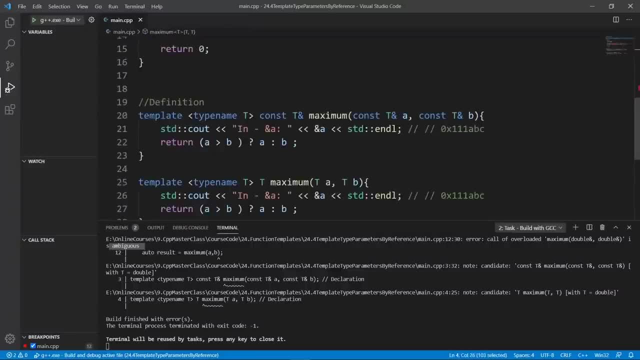 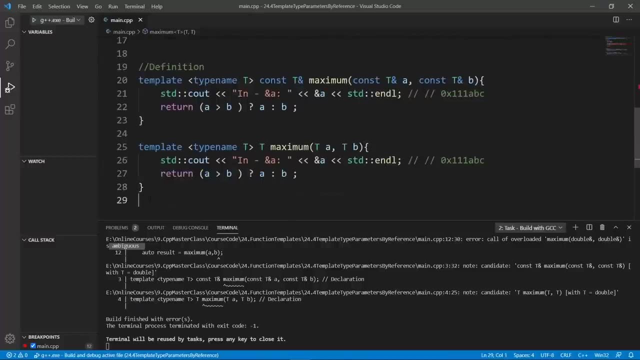 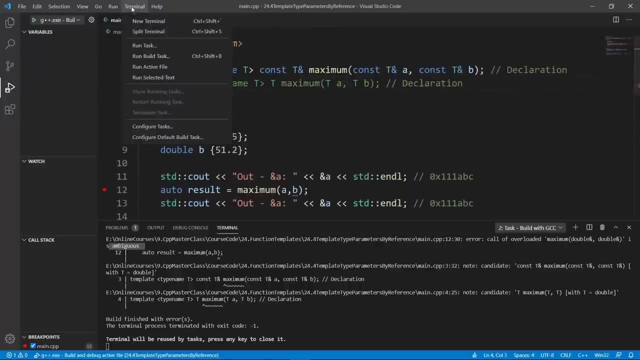 so the compiler is going to give us a compiler error and we have no choice but to use either of these two. but we can't have them all in our code and for example, if we take out the one by value here and leave in the one by reference. so let's comment this out again: if we're bold, we're. 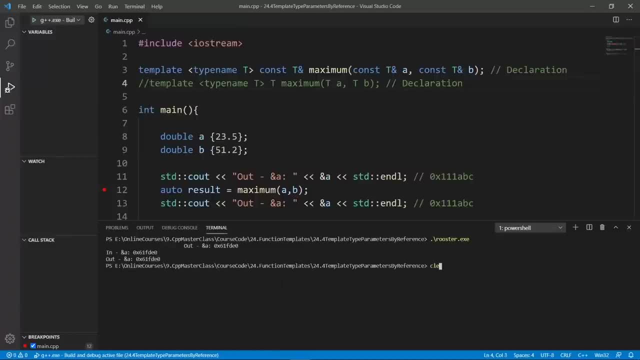 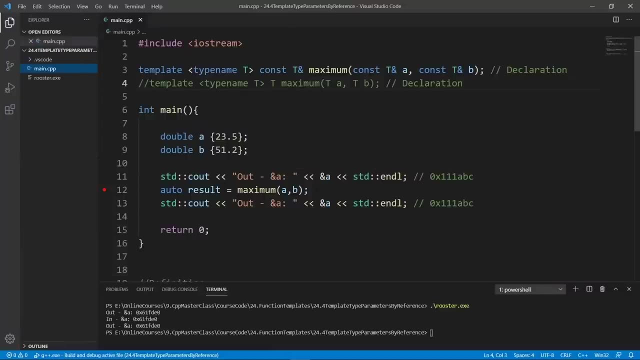 going to bolt. you see the world is good and we're going to print our data however we have it in our code. we see the addresses are the same, and another thing i don't think i really proved to you is that we are passing by cost reference here. so the template instance that is going to be 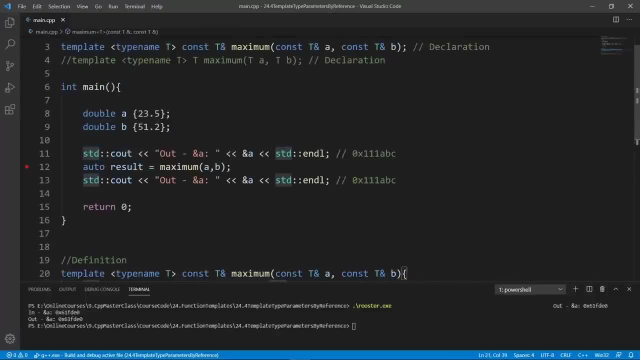 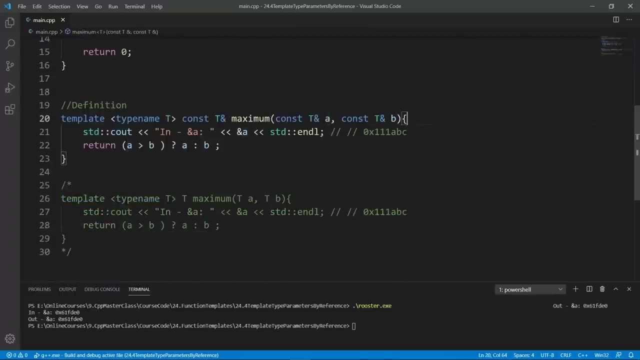 generated is going to be passing by cost double reference because we are passing in double parameters. but because of this cost in front of our arguments here, we want to be able to modify the data referenced by this name here, if we go inside, for example, and say plus, plus a. 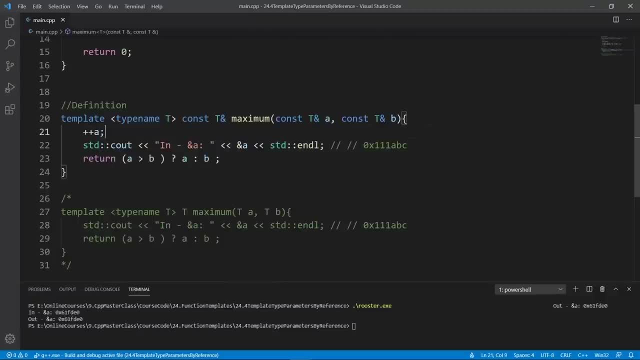 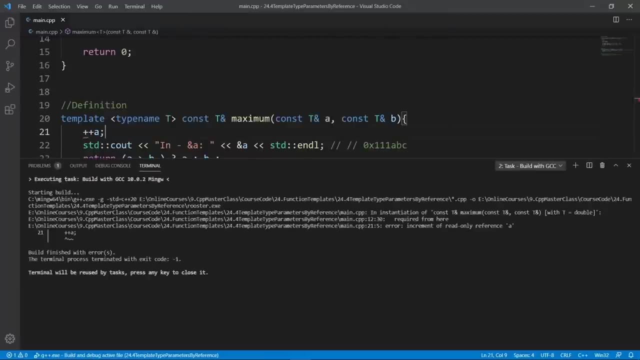 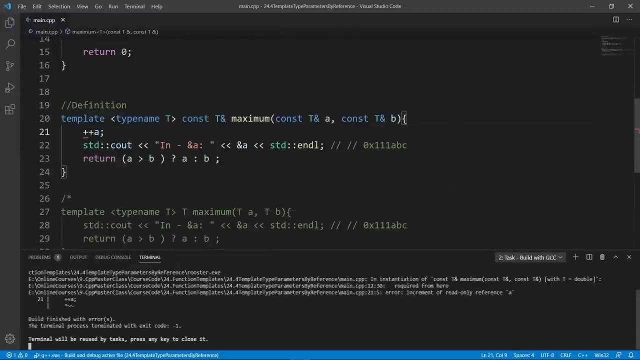 try to modify a in any way through this reference, we're going to get a compiler error. let's work again and we're going to see that and world finished with an error. and it is saying: increment of read only reference a, because we are passing by cost reference here. so you should really remember. 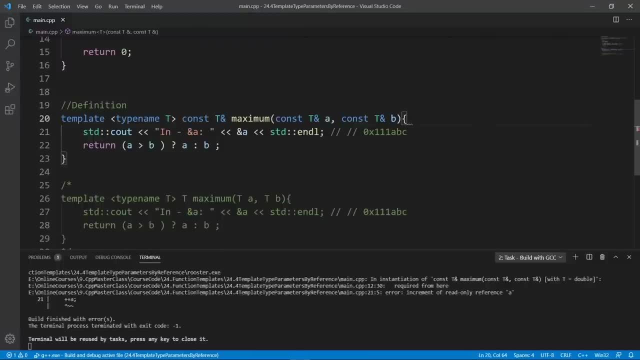 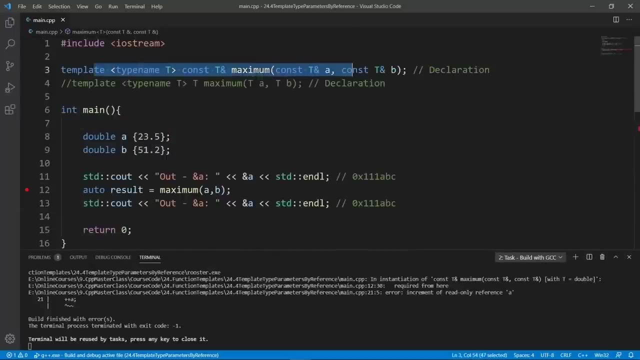 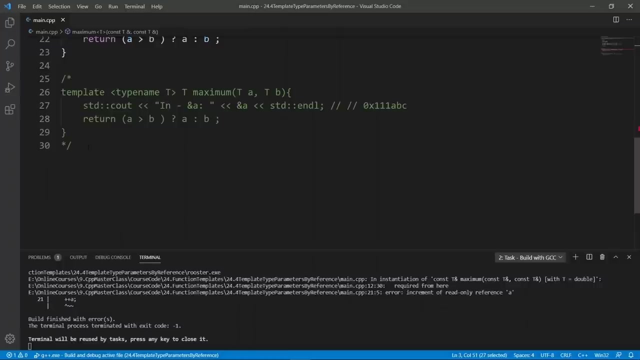 this, even if we are doing things in the context of function templates. this is really all we set out to do in this lecture: showing you that you can set up function templates, take parameters by reference and contrasting this with passing by value and seeing the differences between these two things. we're going to stop here in this lecture and the next one we're 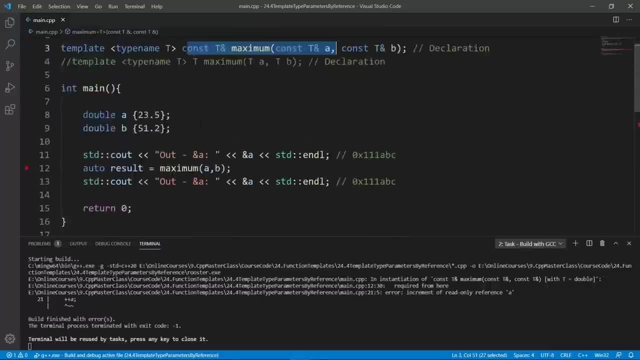 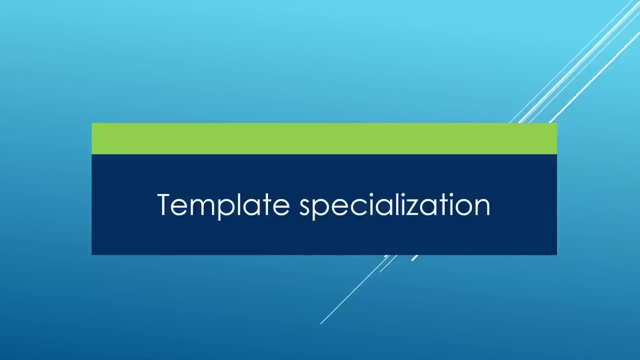 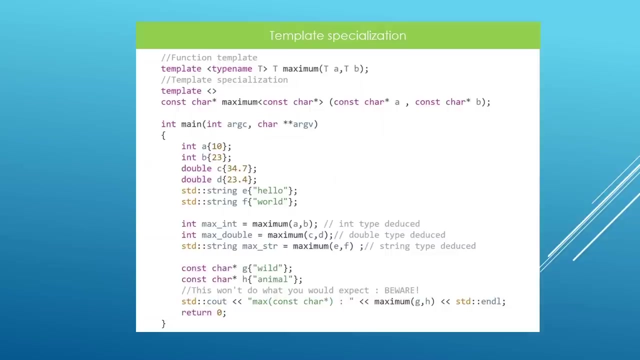 going to learn about template specialization. go ahead and finish up here and meet me there. in this lecture we're going to learn about template specialization and this is a feature we have in c plus plus to bypass the default mechanism of how function templates work in c plus plus. 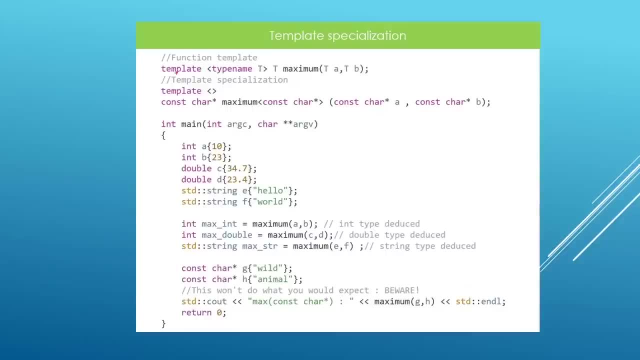 okay, let's make myself super clear. here we have a simple function template. we have seen a thousand times by now. it is the maximum function and it is going to compute the maximum between a and b here and it is going to return that it is a function template. so if we pass in a and b, which are of 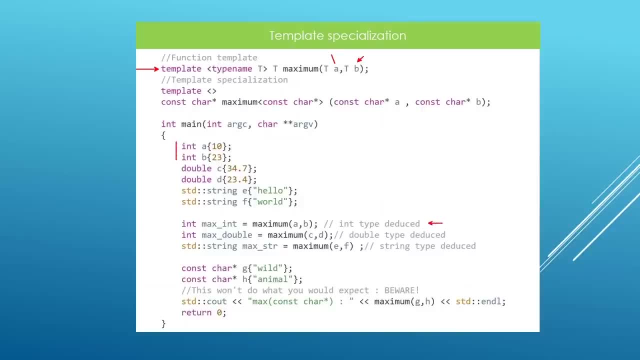 type and we're going to generate a net instance of the template here. if we pass in c and d of double type, we're going to generate a double instance of the function template here. if we're passing std string parameters, we're going to generate an std string instance of this template. 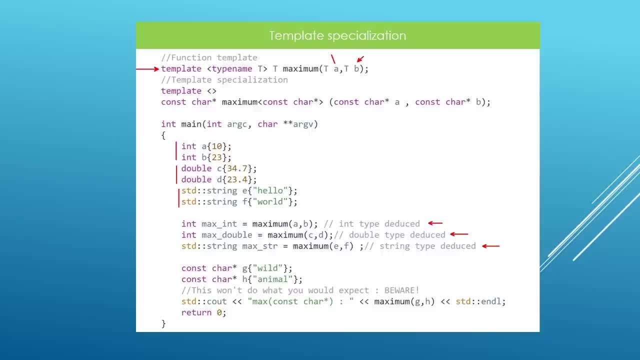 here, and this is going to basically be comparing the parameters we pass. so we're basically going to say if a is greater than b, then return a. if a is not greater than b, then return b. okay, that's going to work if what we're doing is what we have here, but the moment we pass 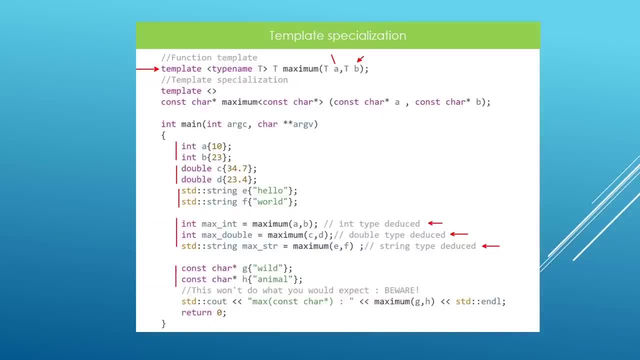 something like what we have here- cost car pointers- then we're going to have a problem because we're going to be calling our function template with cost car pointer parameters. the default mechanism is going to deduce a template instance that works on const car pointer arguments here and what we're going to be comparing now are going to be pointers to the 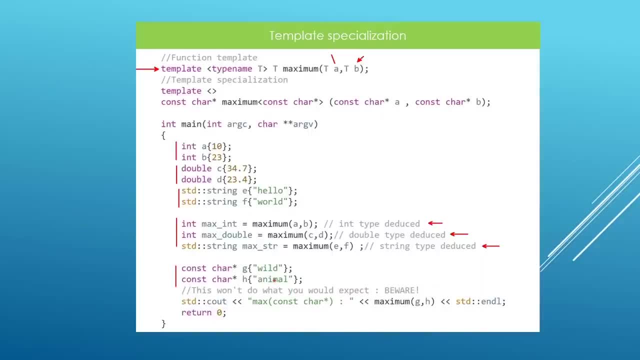 string rather than the string data itself, and hopefully you can see that this is going to be a problem. template specialization is a mechanism we have to tell the compiler for a template function. if i pass you this type, please don't do the default thing you do of replacing in the argument type for the template parameter. instead, use the. 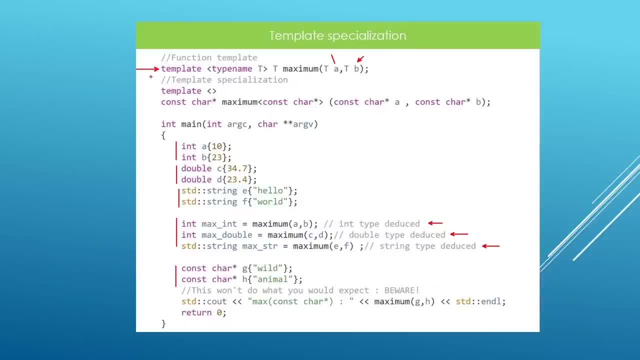 implementation that i am going to give you and you tell that to the compiler using the syntax we have. here you put a template keyword. here you put an empty pair of angle brackets and then you specify your function the way you want it. you see, it's going to be a function that is going to be a. 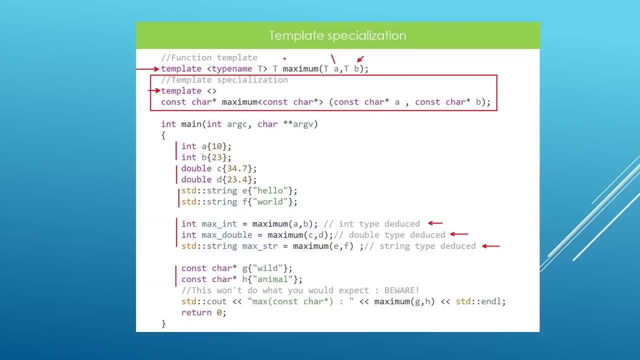 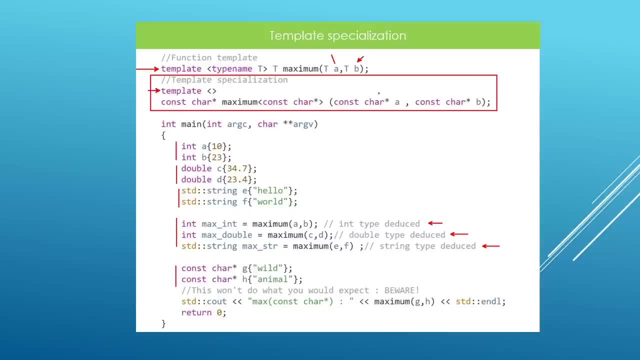 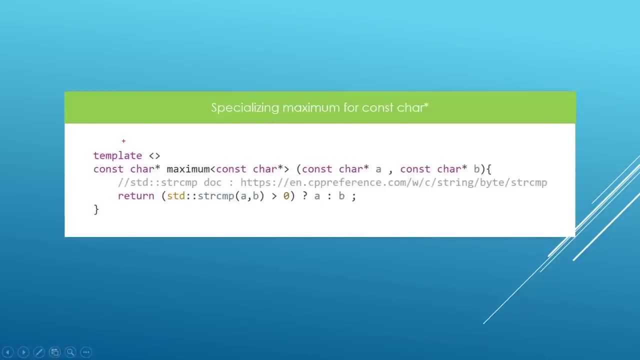 template argument here, and then we pass our parameters, which are also of const car pointer, and when we do this, then we can head in the body of the function and do the comparison however we want. okay, so how do we this comparison here? here is a simple implementation of the function template. 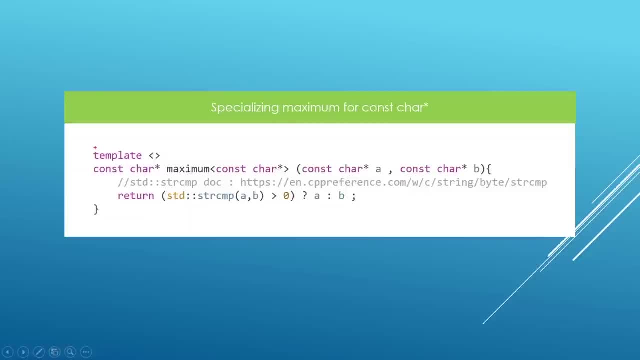 we just saw in the previous video. so we're going to do a simple implementation of the function template. so on the previous slide you see that it really is the same thing. we have the template keyword, we have our angle brackets and we have the function header. here it's going to return const car pointer. 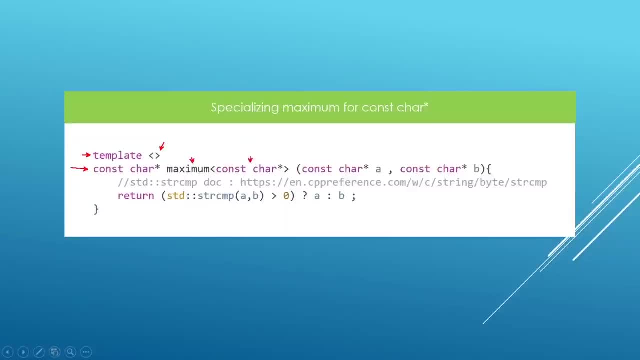 it's going to be called maximum and an explicit template argument is specified within these angle brackets, and then we have our parameters. what is really important about this function is that it's not going to do the comparison we've been doing all along. it's going to use a built-in function. 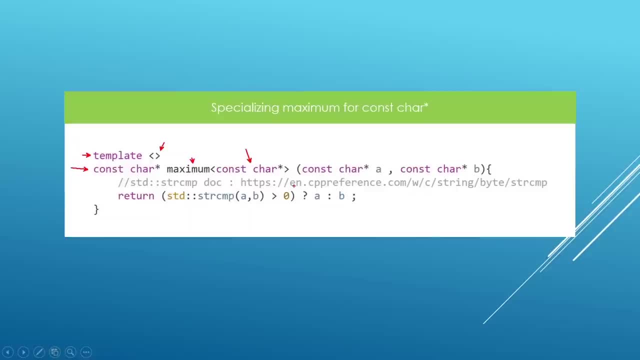 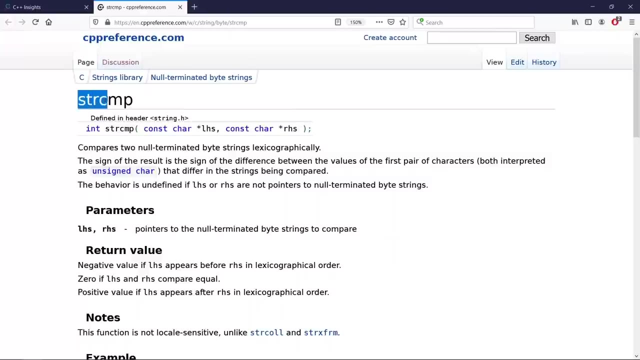 in the c++ standard library, which is specialized for comparing c strings. okay, if we come at cpp reference here and look at a function called strcmp- we have seen this before, i guess- it is going to compare two null terminated byte strings lexicographically. and you see, this is really what. 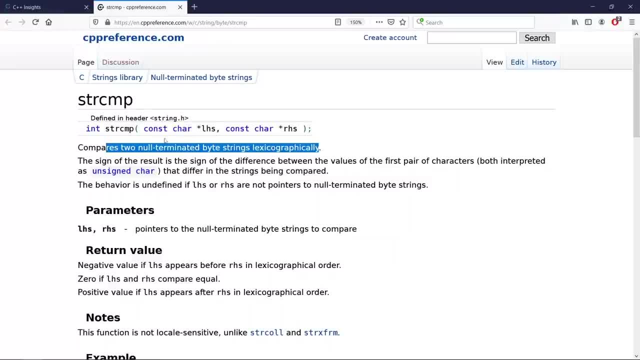 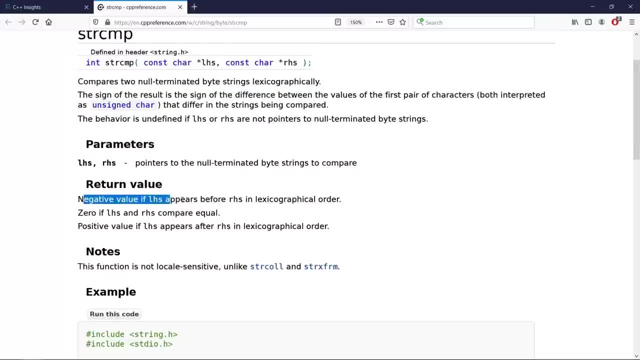 we want. we have two const car pointers. one is going to be the first parameter, the other is going to be the second parameter. we're going to compare them and look at the return value. we get a negative return value if the first parameter comes before the second parameter. in lexicographical 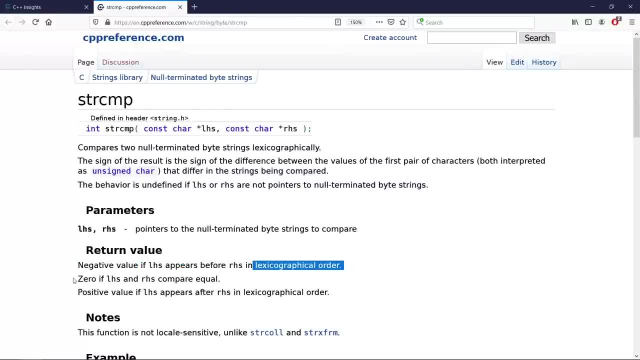 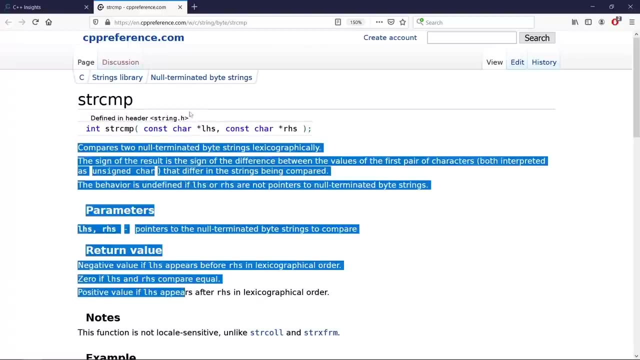 order. we're going to get a zero if they are equal and we're going to get a positive value if the first parameter comes after the second parameter in lexicographical order. so we're going to use this information here and compare our two c strings here and return something in visual studio code. 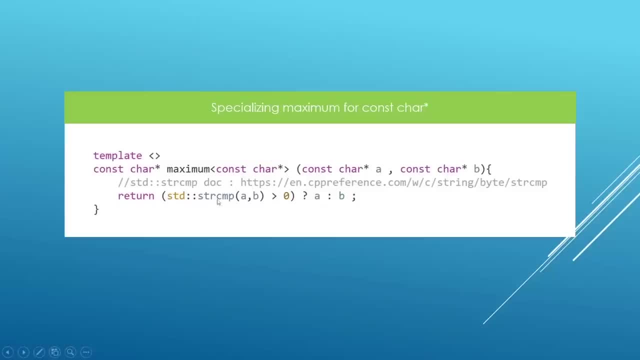 okay, so this is the function here. it's going to compare the two c strings here and return something in visual studio code. so we're going to be using the logic from strcmp and notice what we return. we're going to return whichever string compares greater to the other. so we're going to do strcmp. 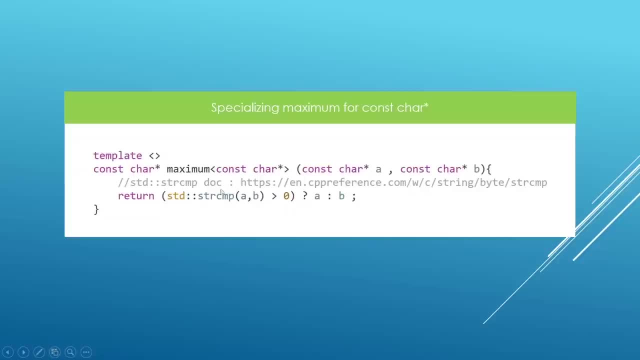 we're going to pass in our two arguments here and we're going to say: if this returns something greater than zero, return a, because in that case a is greater than b lexicographically. this is the comparison we want to do here, and otherwise you're going to return b and this is going to compare our. 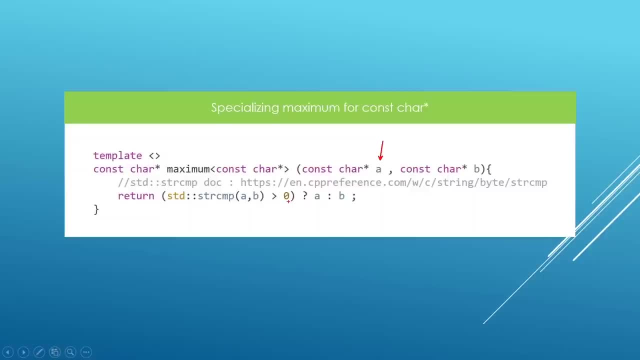 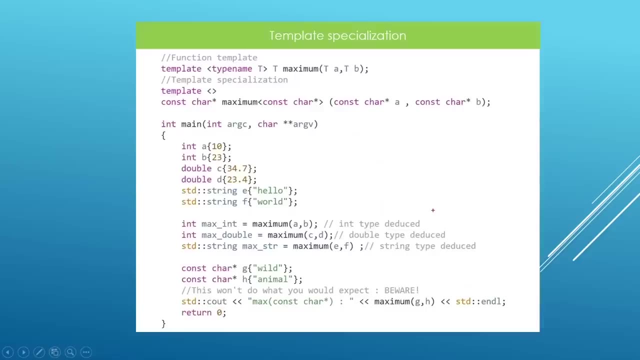 not compare pointers directly, which is what we are trying to avoid here. and you see that template specialization is really helping out here. now, if we have this in and the compiler sees a call like this, it's not going to compare pointers, it's going to use the template specialization. 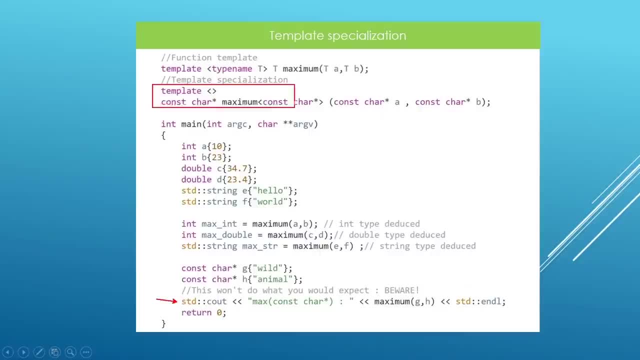 because the compiler knows that this is a better fit for the call that we are doing here because we are passing const car pointers. this is how template specialization works and it can really come in handy if you are doing things that work with pointers. we are going to. 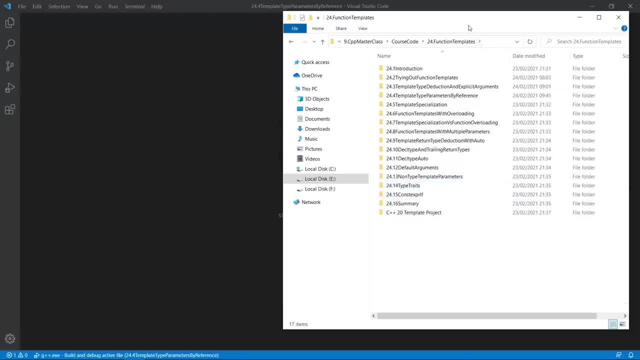 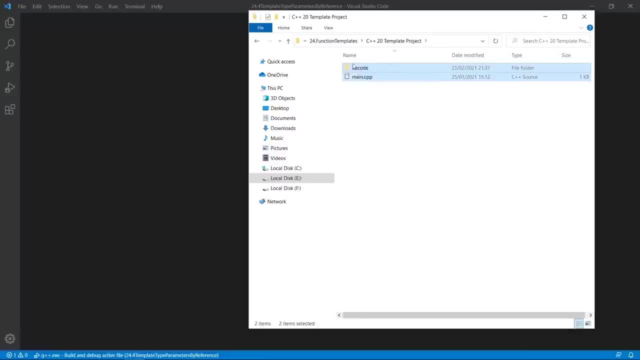 head over to visual studio code and play with this a little more. okay, here we are in our working folder. the current project is template specialization. we're going to grab our template files, we're going to put them in place and we're going to open this in visual studio code by dragging. 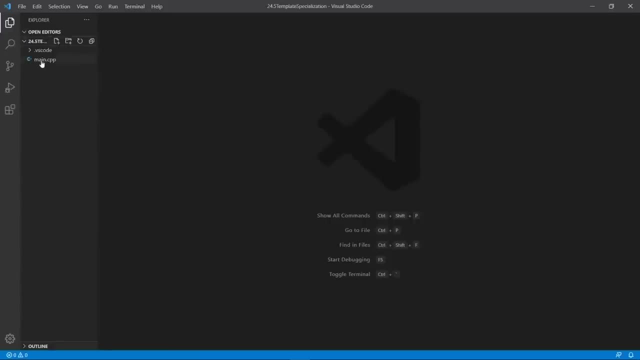 and dropping on top of visual studio code here. this is going to open our project and we're going to close it a little bit and we're going to close the left pane here. we don't need it anymore. the first thing we're going to do is to put in our function template the same thing we have been. 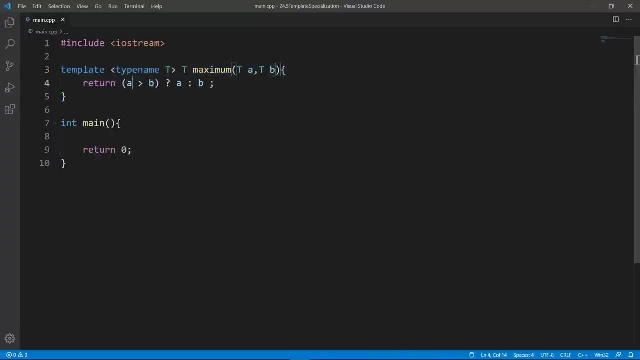 doing for a gazillion times by now. the maximum function: it's going to return whichever is greater between a and b, and it is doing this by value. after that we're going to head over in the main function and set up a piece of code to really play with us. we're going to set up a few variables. 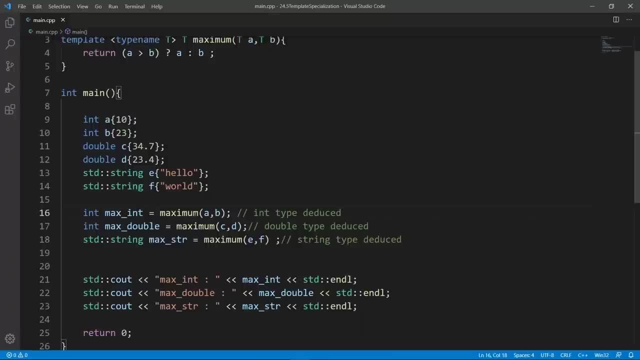 and we're going to call our functions: say, maximum a and b. this is going to return the maximum between a and b. the compiler is going to deduce that the template instance should be of int type, so it's going to generate that and call it. it's going to give us the return value here. we can print it out and see it and we're going to 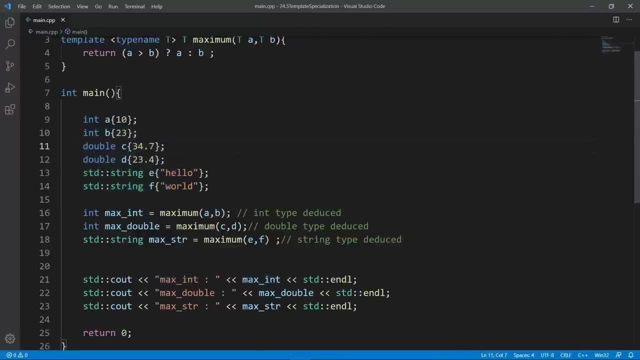 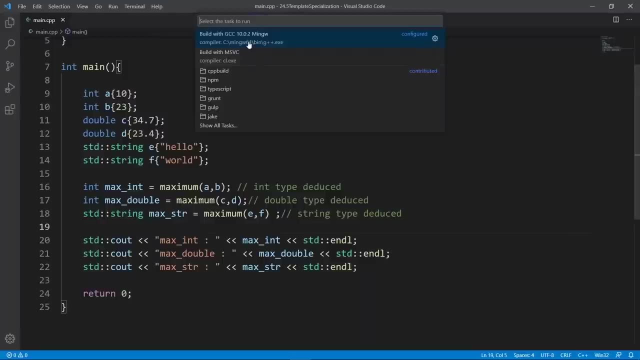 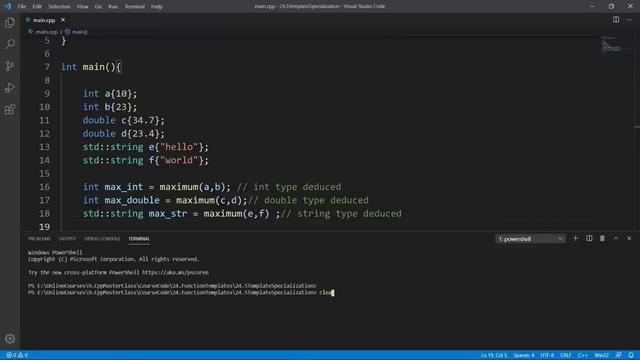 basically do the same for double type and string types here, and you're going to see that this is going to work just fine. so let's build this. we're going to use gcc to do that. the build is good. we can clear and bring up a terminal to run this and really see the output. here we can clear and run. 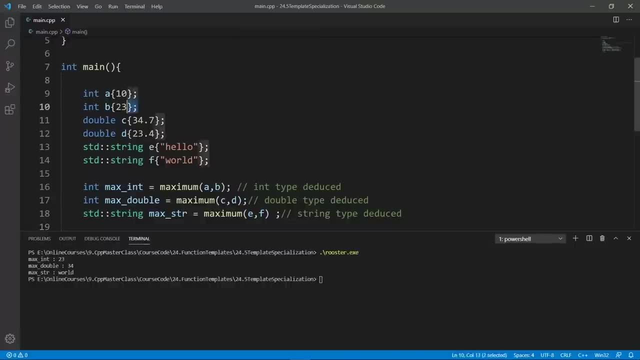 rooster. you see, max end is 23 because that's what we have here, max double 34 and that's what we have here and we called max double to be of end type. we should use auto type deduction here to avoid these mistakes, because the compiler can do this better than us. that's what we're going to do and we're 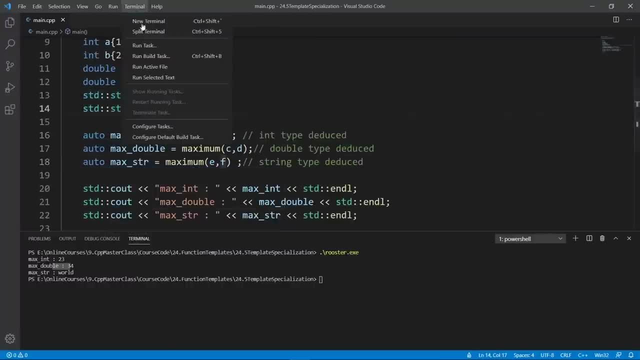 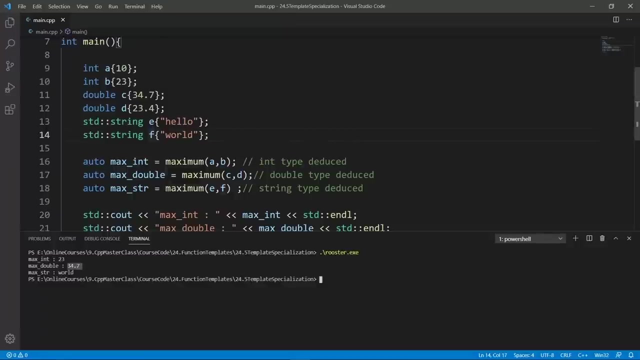 going to deduce max str here and we're going to build again. let's build with gcc, because that's my favorite compiler. i'm going to clear and run rooster. now we have correct output. we have 23, which is the maximum between a and b. we have 34.7, which was deduced to be of type double here, and then we have the maximum strength. 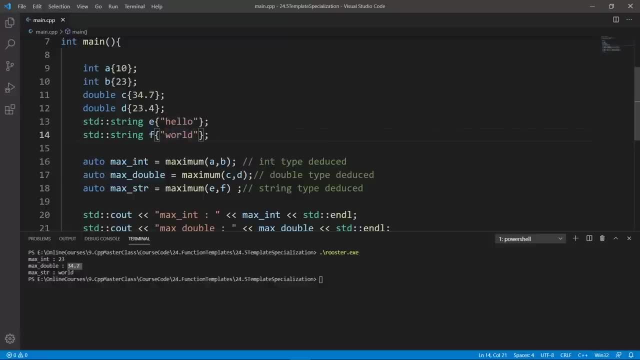 which happens to be world. here again, when comparing strengths, the default is going to compare them lexicographically, and what that means: the one that comes after the other in alphabetical order is going to be greater. by that logic, world is greater than hello, and it is what we are seeing printed out here. okay, this is working. 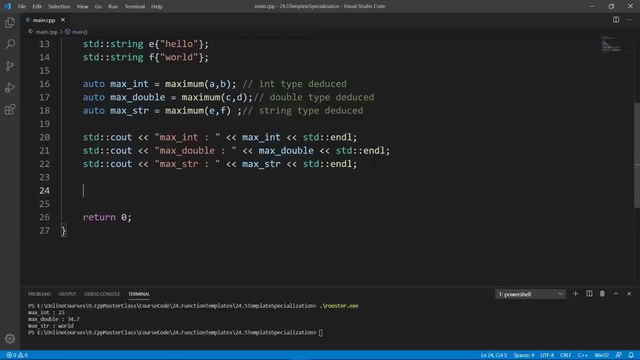 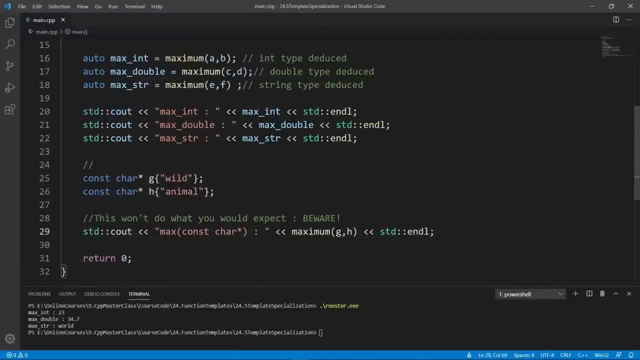 just fine. but what if we use const car pointers and try to call our maximum function template, and by that i mean doing something like this: we have two variables, g and h, which are of type const car pointer, so they are c strings. they are going to be. 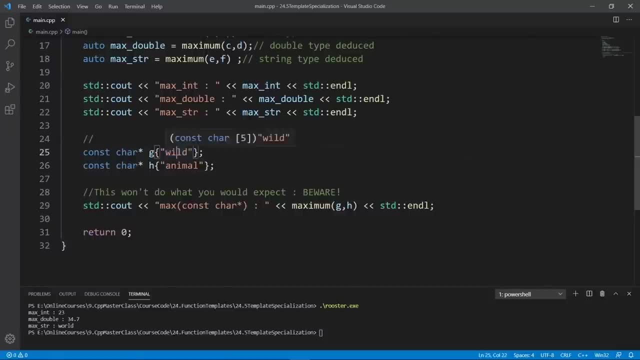 now terminated, because we are initializing them with a string electron and we are comparing them here. we are saying maximum g and h and we're going to print whichever is the maximum after we return that from the function. when the compiler says the call like this, it's going to do what it. 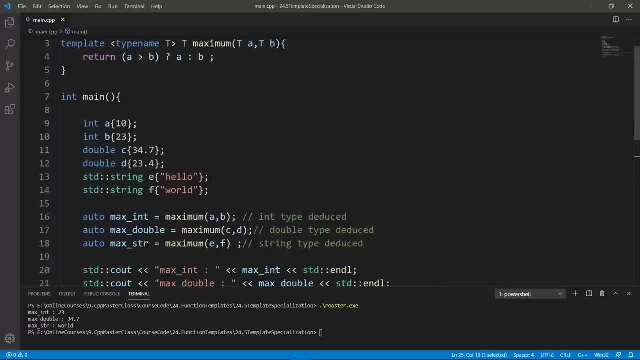 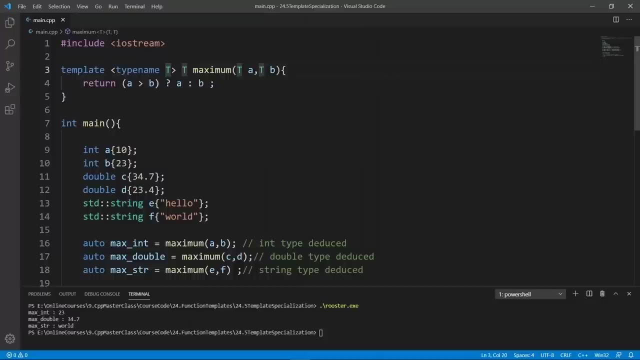 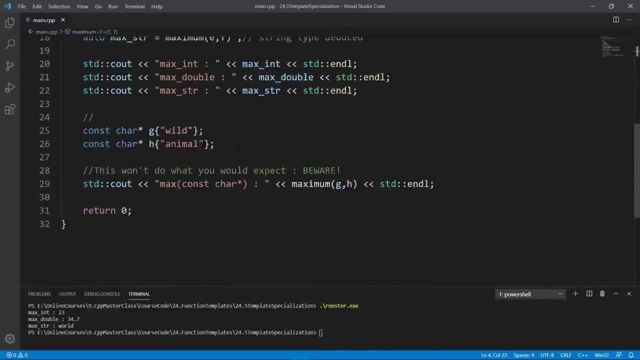 knows to do. it's going to replace an const car pointer in our function template here, so it's going to return const car pointer. it's going to pass the parameters as const car pointers and we're going to be comparing these pointers here and we're going to return whichever pointer is greater. again, here you must be noticing the. 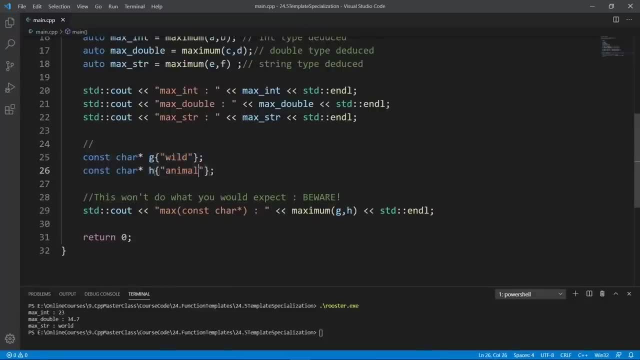 problem. we're going to return whichever pointer is greater, and we're not going to be returning the actual string data. we're going to be returning just the address, and this can be really wrong, because if the addresses happen to be messed up, we're going to get the wrong output. so let's try. 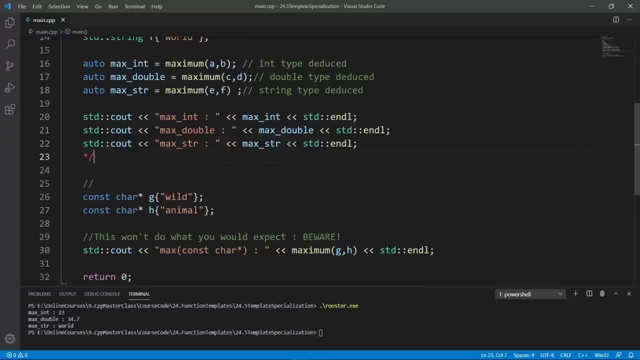 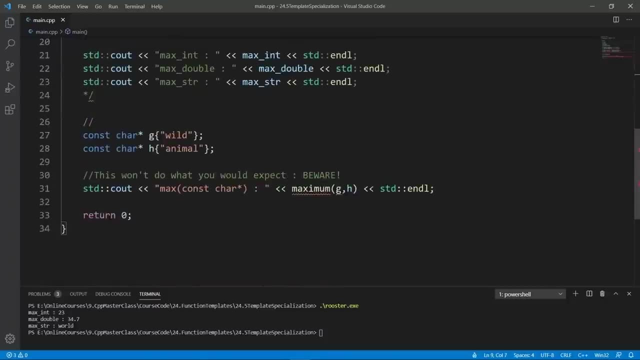 and prove this again. for that i am going to comment out what we had on top here, because this could mess things up a little bit. so i'm going to comment all this out and i am going to debug this. so we're going to look at this line here and i think we should say const car pointer. 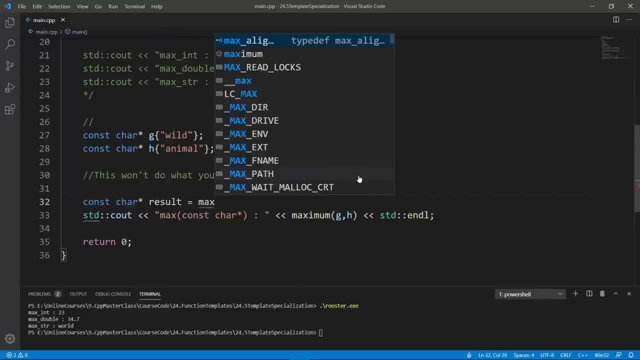 result and say: equals maximum g and h. and i printed the result here. this is going to make it easier to step into this function without the noise from stdc out here. so we're going to set up our break point here. we're going to hit our 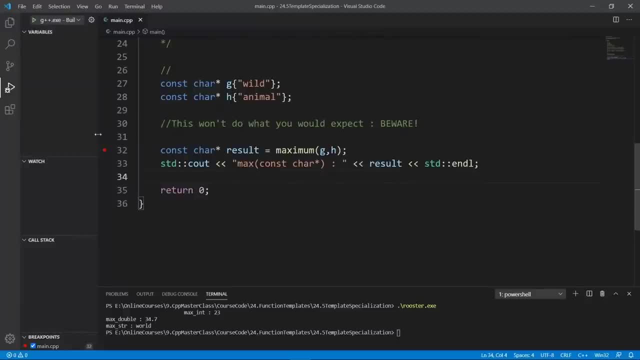 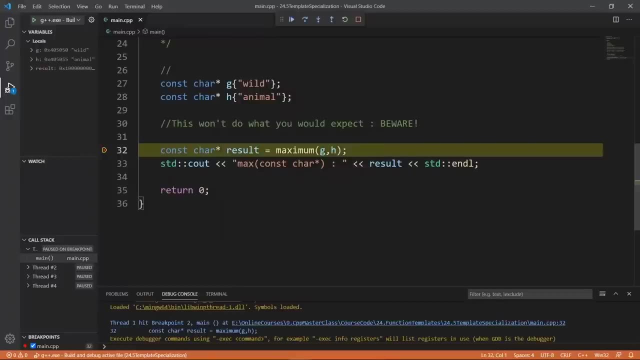 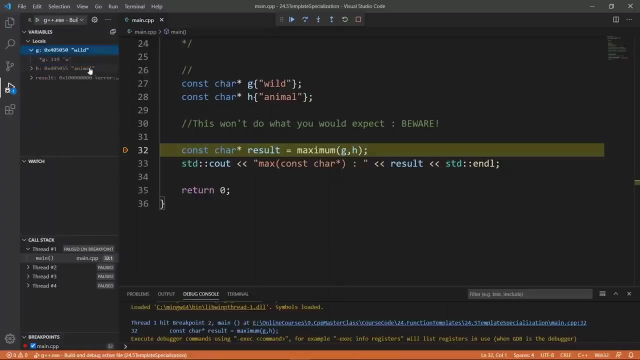 run tab and we're going to debug this program and we're going to hit this break point here. let's see the types that we have inside our function call. so, now that we are here, we're going to see that our locals are g and h and they contain our string. if we go inside, we're going to 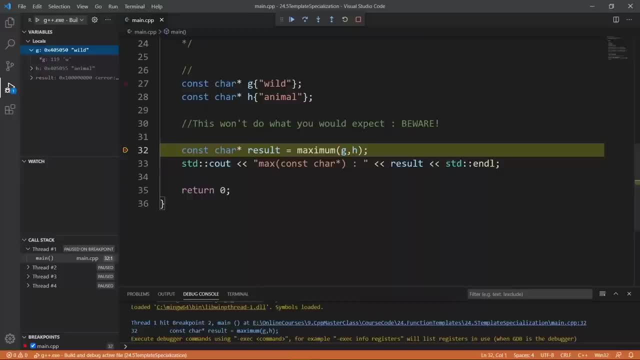 see that g is really a pointer to the first element in our string here and it contains w here and h is going to be a pointer to a. that's what we have here, okay, and result is going to contain some junk data because it's not initialized yet. but we can step into this function and see things. 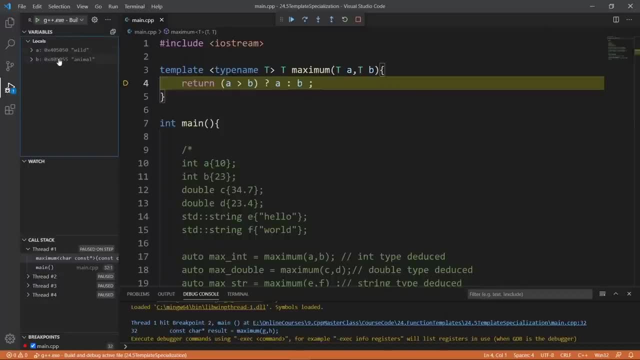 happening. a, again, is an address and b is an address. you see that the debugger is really smart. it's noticing that this is a pointer to a string and it's going to show us the string here. but what we compare are these two addresses and you see that b 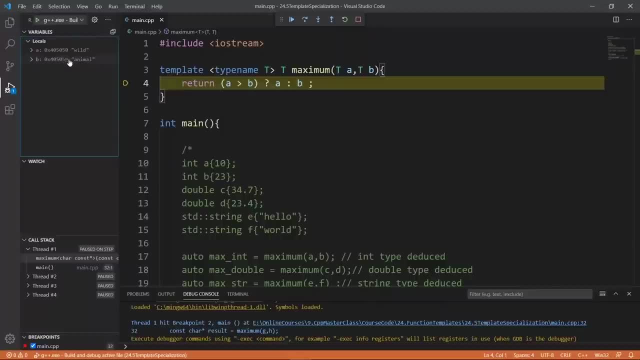 lives in a larger address, it leaves at address that ends in 55 and a lives at the address that ends in 50. so if we really execute this function, we're going to return the pointer to b, but you see that b is not really the greater strength and this is really something bad you should be aware of. 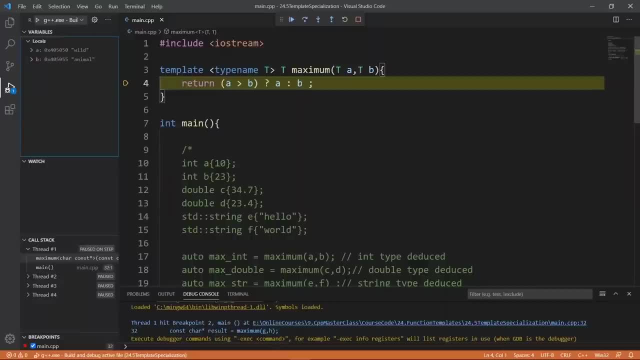 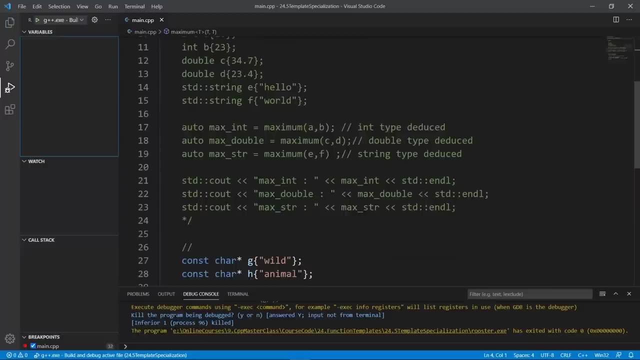 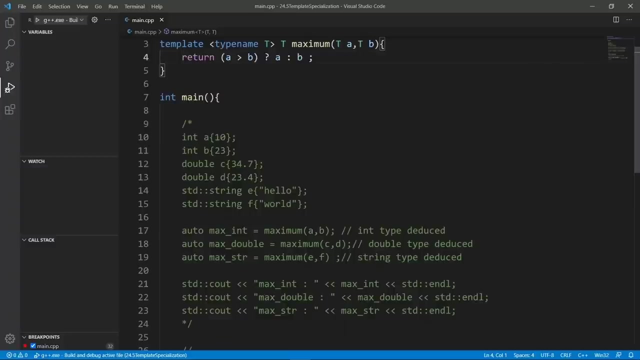 this. this is what the compiler is doing by default, and it is going to give us a result that is not correct. let's close this and see a way we can solve this problem, and we can use template specialization for this. what we really need is a way to compare c strings and not compare pointers. 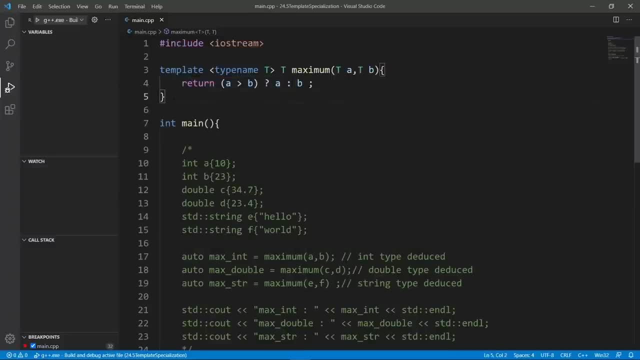 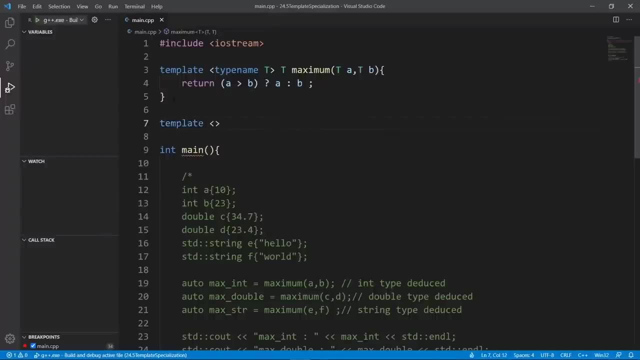 like we are doing here. we're going to do that using a template, specialization and the syntax for this to work, you say template and you specify an empty pair of angle brackets and then you specify whatever function you want to use. so we're going to go down here and specify that we want to. 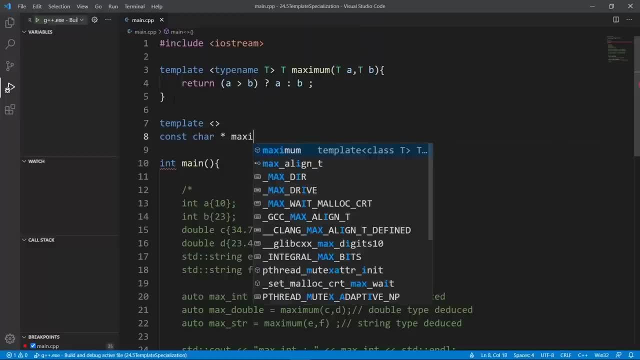 return a function. in the grammar it will export to donkey對啊 represents the order of theала punch. mentioning const car pointer, the function is going to be called maximum. we're going to specify an explicit template argument which is of const car pointer, because we want this template instance to work. 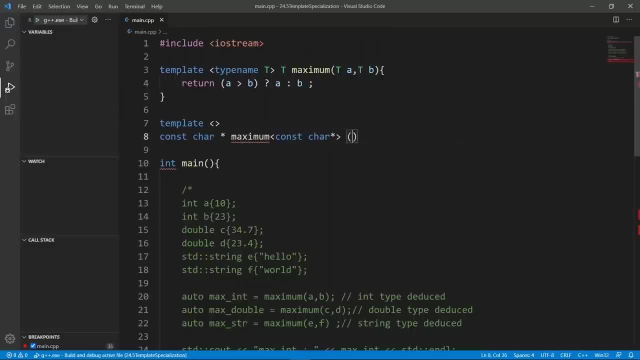 for const car pointers. so once we have this end, we're going to specify our parameters. we're going to say const car pointer a and const car pointer b and we're going to head into the body of our function template here. now we have our two parameters and we're going to compare them as 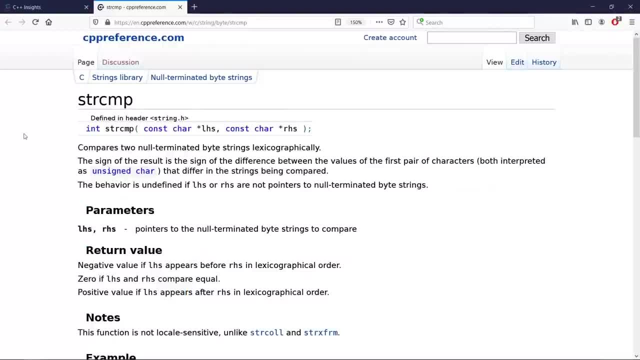 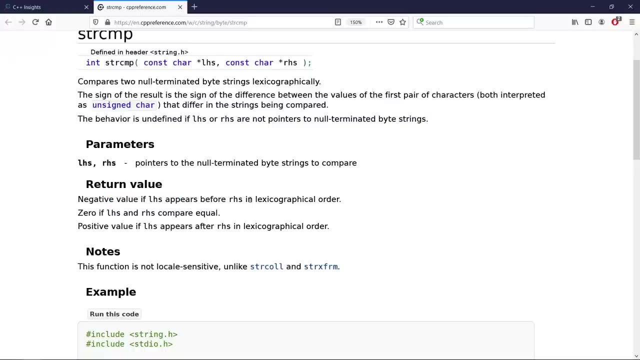 if they were const car strengths. and we have seen that we have a built-in facility from the c++ standard library. it is this strcmp function. we can use it to compare two strengths and we're going to use the logic that we have here. so if the first parameter is less than the second parameter, 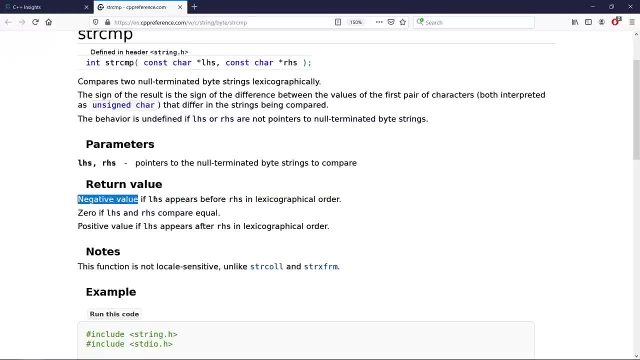 i am talking in a lexicographical order. we're going to return something negative. if they are equal lexicographically, we're going to return zero. and if the first parameter is greater than the second parameter, lexicographically, we're going to return a positive value. so let's transform this logic into a ternary. 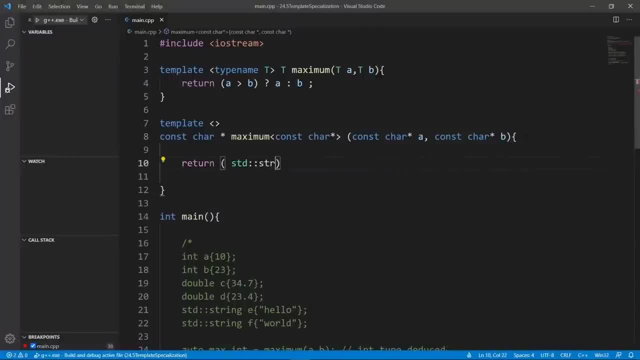 operator. we're going to say return std str- cmp. we can say that, and to have access to this function, we're going to need to include c string. let's do that. we're going to include the c string library and in our case we're going to say return std str- cmp and we're going to say return std str- cmp. 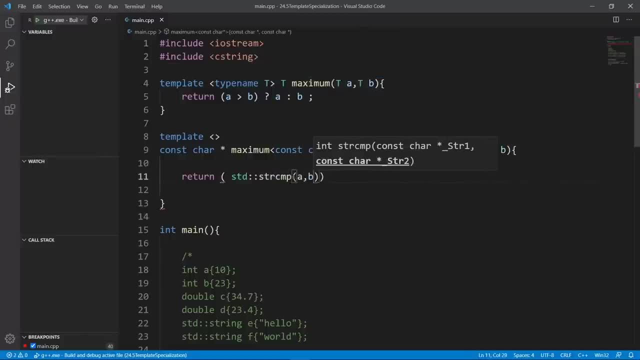 now we can say this and we're going to pass in a and b and we're going to ask ourselves: is this greater than zero? okay, if it's greater than zero, then the first parameter is greater than the second parameter lexicographically. so we're going to return a. if it's not the case, we're going to 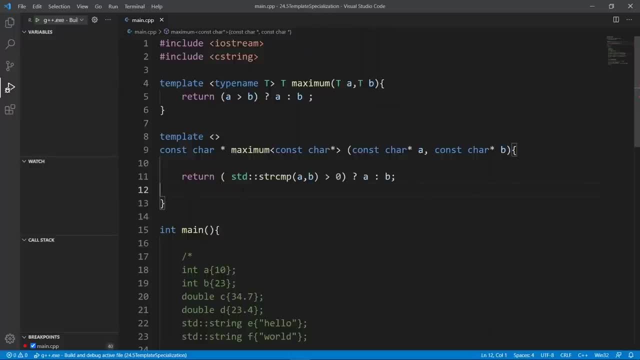 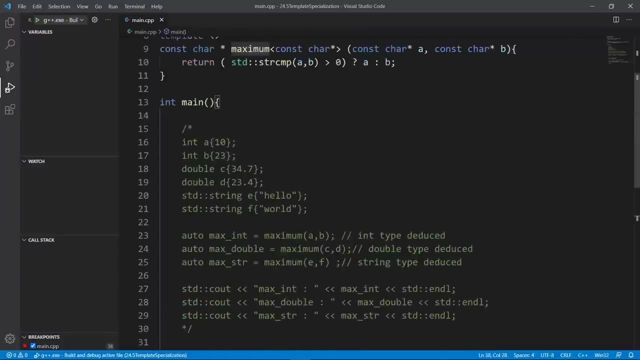 return b. this is our ternary operator here and it is going to work. now that we have this n, the compiler is going to know we have a template specialization for const car pointer. if the, if we call the function like we did here, calling the maximum function, the compiler is not going to. 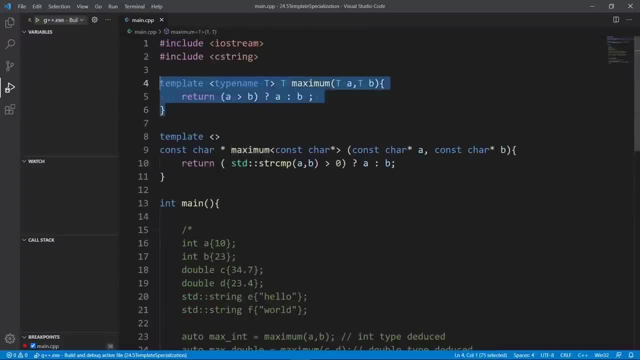 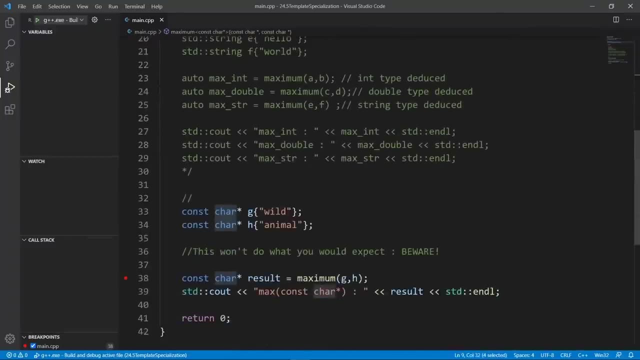 use this function template we have on top here. it's going to see that this template specialization is better for the const car pointer type that we are passing here and now. if we try to build and run the program, the build is going to be good. if we clear and run rooster, we're going to see that. 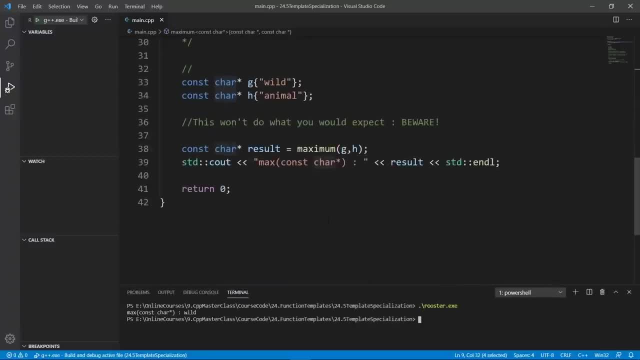 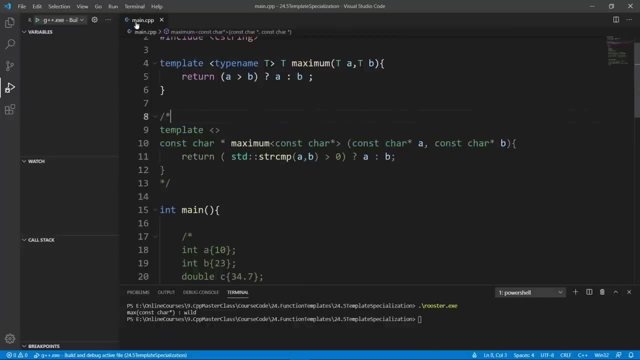 now the maximum is wild. let's see what we see. if we don't have this specialization- and we're going to comment this out because i don't think i really showed you- we're going to build again and again. if we do this, this function template is going to be used and you. 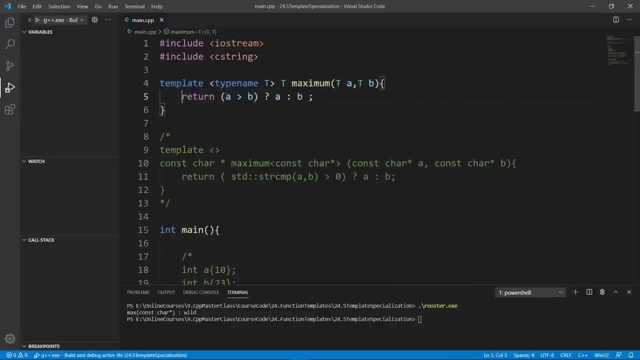 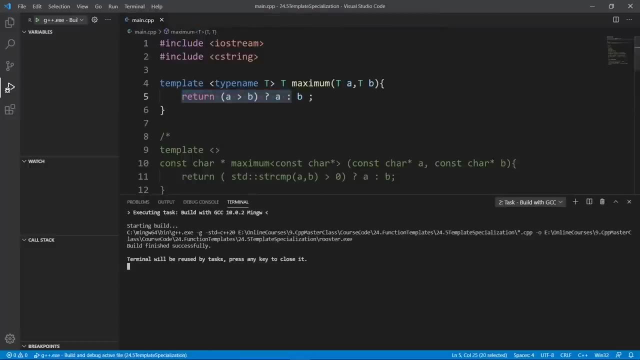 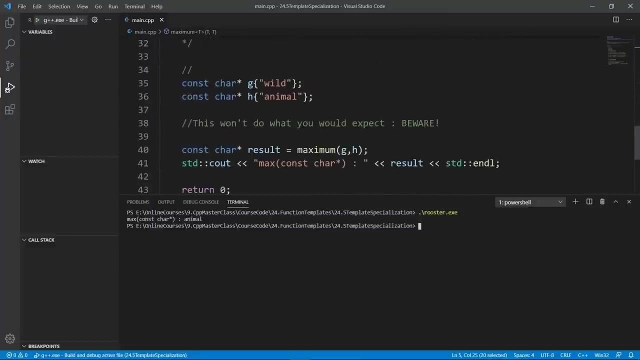 know that it is going to deduce a function that compares pointers directly and that's going to be really bad. we can world this with gcc and really see what we get as output. we can clear and run rooster. now you see that we are saying animal is the maximum between these two guys. but that's not. 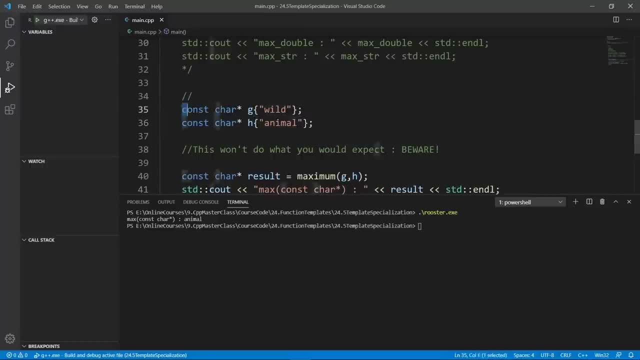 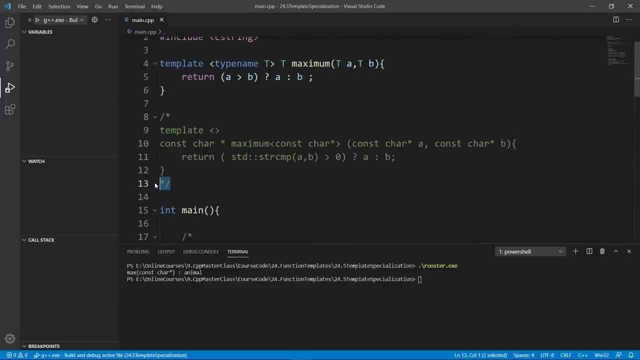 true animal is less than wild in lexicographical order. we need a way to really compare c strings properly and our template specialization is really doing that using the std crmp function and it is working pretty well. this is really all template specialization is all about you're going to do. 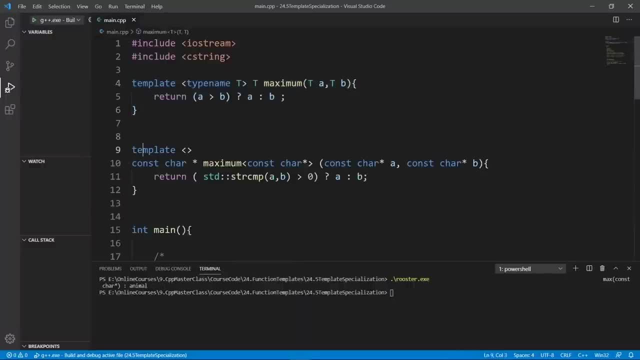 this if the default function template you have is really not working according to your needs for the function you want to use. for this, and use this to your advantage because it's available to you and now you know how to use this. the syntax is really simple: you say template and you say angle brackets. 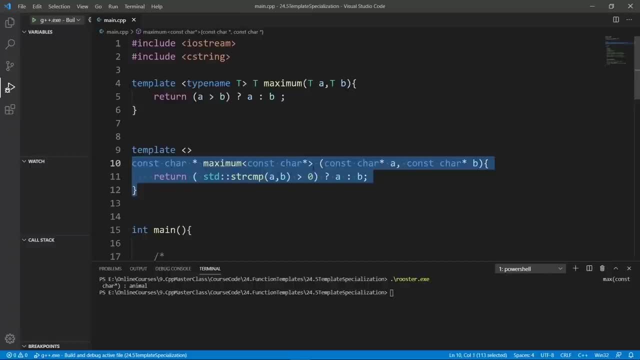 and then you specify whichever implementation you want for your specific type. for example, here: our specific type, for which we want to specify this function template, is cost car pointer. you specify that as an explicit template argument and then you specify your return value, your, and you do whatever logic you need to do to do things right in the body of this template specialization. 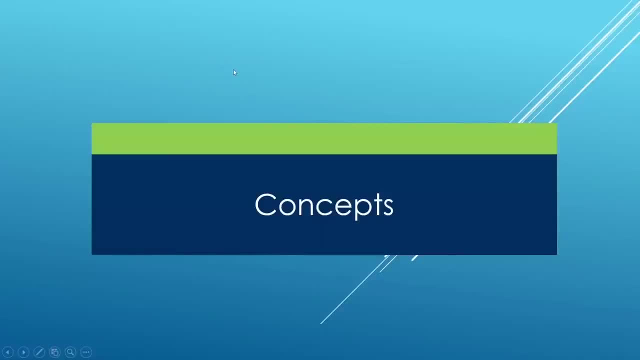 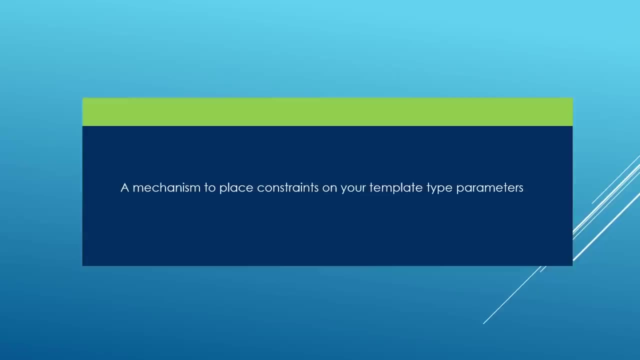 here. i would like to welcome you in this new chapter where we're going to be learning about concepts. concepts are a mechanism we can use to set up constraints or restrictions on the templates parameters in our function templates, for example. we can use this technique to say that we want our 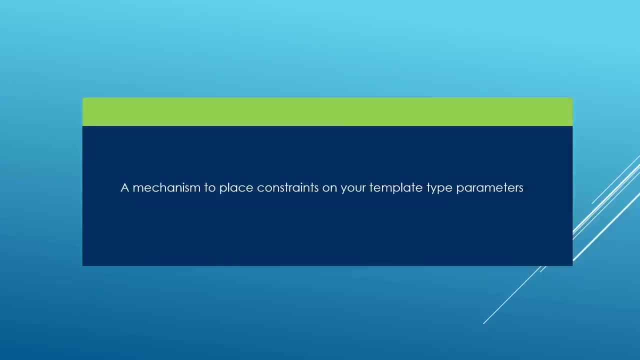 function to be only called with integers, and if you call it with something that is not called with an isn't an integer, it's going to give you a compiler error. one thing i should emphasize is that concepts are one of the big four features in c++ 20, so we're going to be learning about this in this. 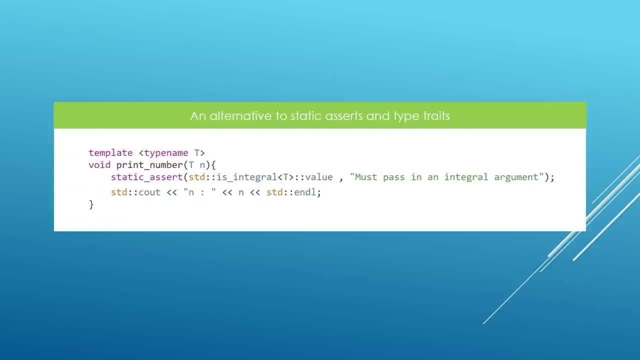 chapter. we have just said that we use them to place constraints on our template parameters. but we saw that we could do something like that in the last chapter, where we could use type traits and static asserts, for example, if you look at the function here, it's going to print a number. 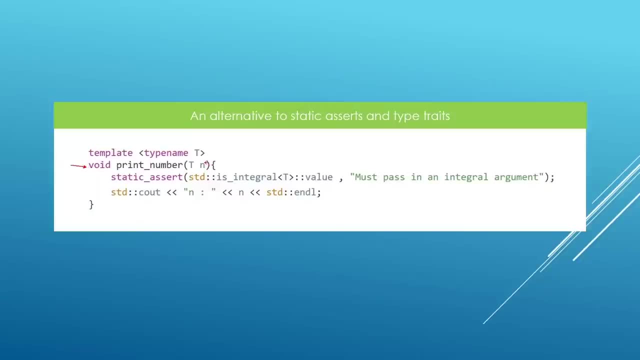 but we have a requirement for this number to be an integral type. through the static assert that we have here, we're going to see that we can do something really similar with concepts, but it's going to be much cleaner, and that the logic to enforce our constraints is not going to be in. 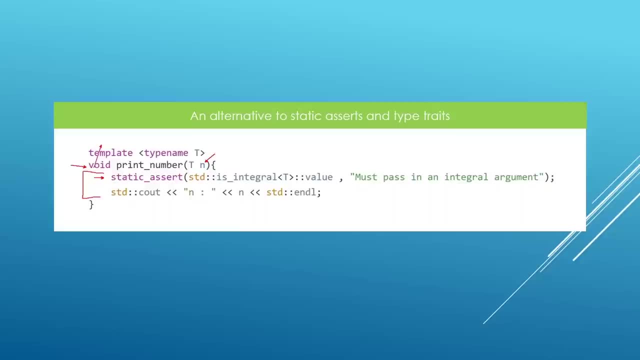 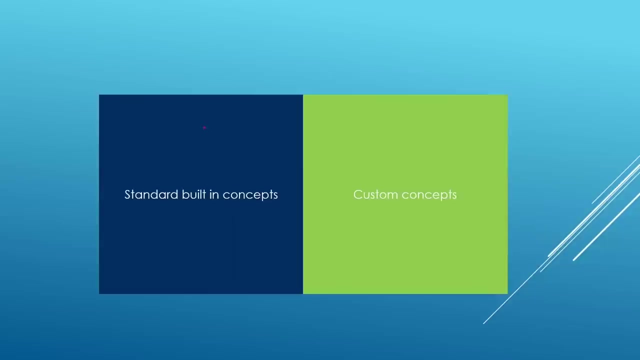 the function body. it's going to be somewhat in the function declaration, in the constraints that we put on the template parameter. here we're going to see specific syntaxes of how you can do that, starting in the next lecture. there are two sides to concepts in c++. there are standard built-in. 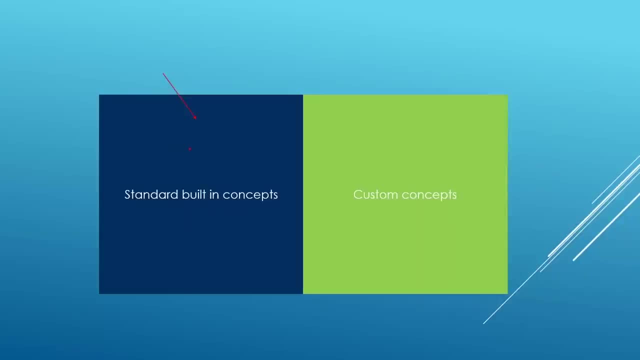 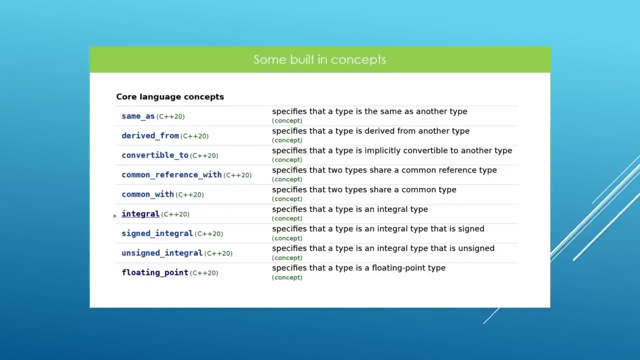 concepts that come with the c++ programming language. but if for some reason, these happen not to be enough, you can build your own, and we're going to see how we can do that later in this chapter. here are a few examples of concepts you can use in your c++ program. you can use the integral. 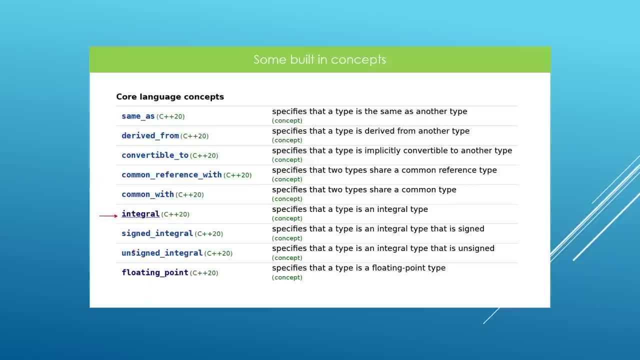 concepts to enforce that your parameters be integrals. you can use the floating point concept to enforce that your template parameters be of floating point type. you can do all kinds of crazy things. okay, concepts are really cool and they are going to make your function templates much safer to work with. we are going to stop here in this lecture. 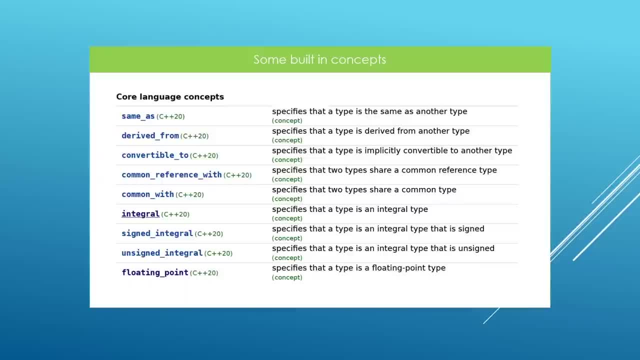 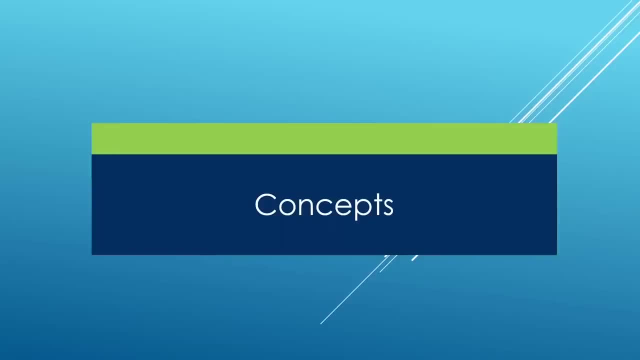 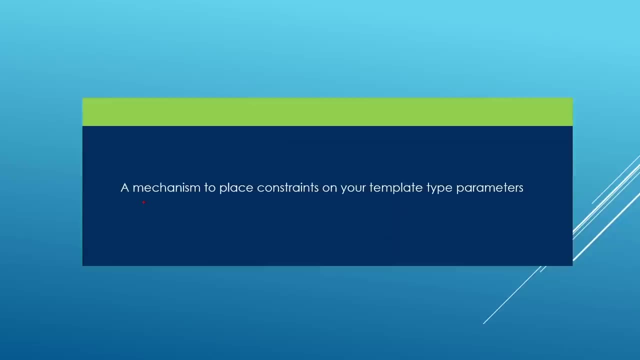 and show you how you can use concepts, starting in the next lecture. go ahead and finish up here and meet me there. in this lecture we're going to learn about concepts again. concepts are a mechanism we have in place in c++ 20 to place constraints on our function templates. for example, we can use: 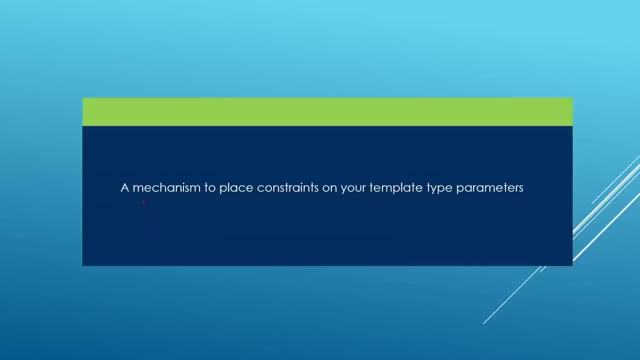 concepts to specify that we want our function template to only be called with integers or doubles or strings or whatever, and when somebody violates our concept they're going to get a compiler error. in this lecture i am going to show you how you can set up your concept and different syntaxes. 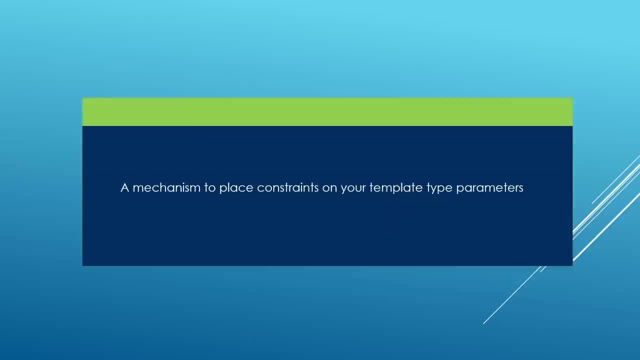 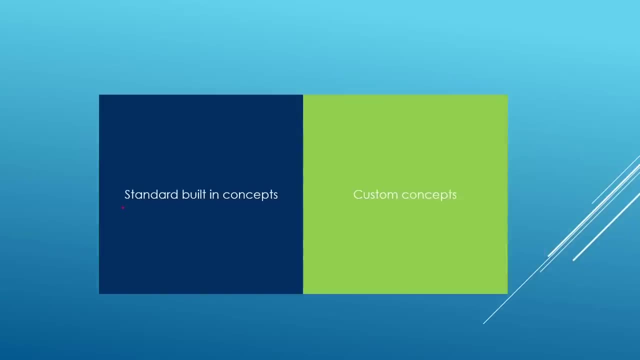 you can use and how we can understand them. but before we do that, please note that there are two sides to concepts. there are concepts that are standard and built into the c++ standard library and those are ready to use, and these are what we're going to be using in this lecture. but know that you can also build your own concepts and use. 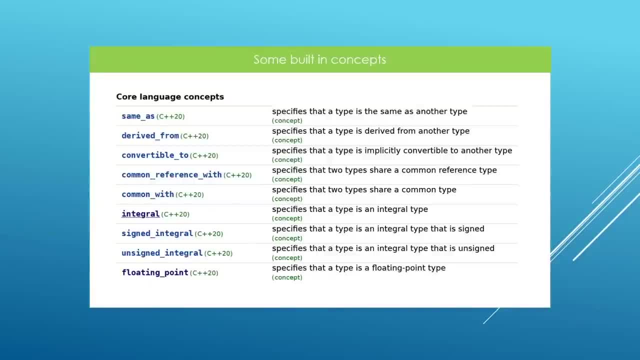 them to do whatever it is you want to do. here are a few examples of built-in concepts we can use from the c++ standard library. we have, for example, a concept we can use, for example, a concept we can use, to enforce that people call our functions only with integral types. if they violate this, they're. 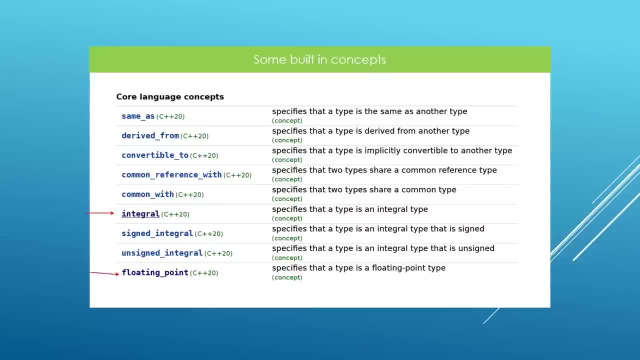 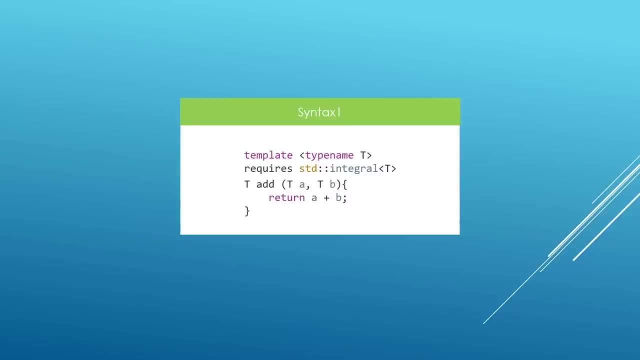 going to get a compiler error. we can also enforce for our template parameters to be floating point. we can do all kinds of crazy things. okay, now that you know this, let's see how we can set up a concept on our function templates. and this is the first syntax we're going to look at all you really have. 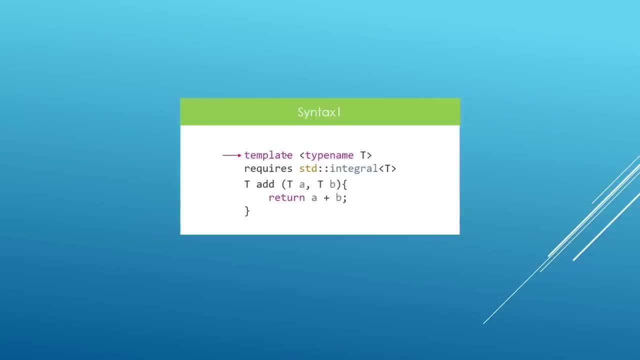 to do is to put in your template declaration, like we have been doing all along, so let's go ahead. and you also have to add in the requires keyword here after the requires keyword, you're going to specify your concept and specify your template parameter in angle brackets here. when you have this thing, 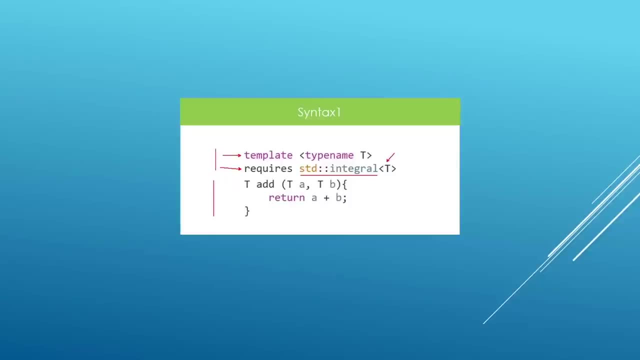 in front of your function template like we have here. the function template can only work right if the concept in here is satisfied, and this concept in this case is going to be satisfied. if somebody tries to call this function template only with integral types, if they violate that, again they. 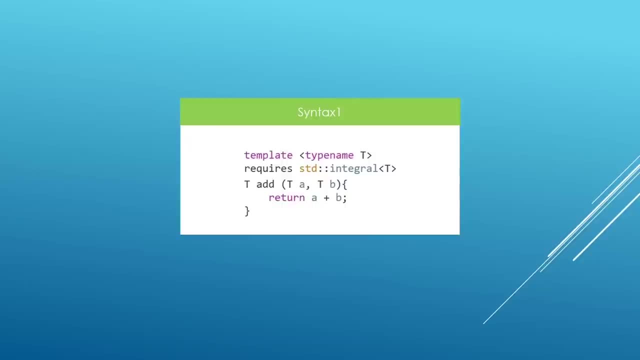 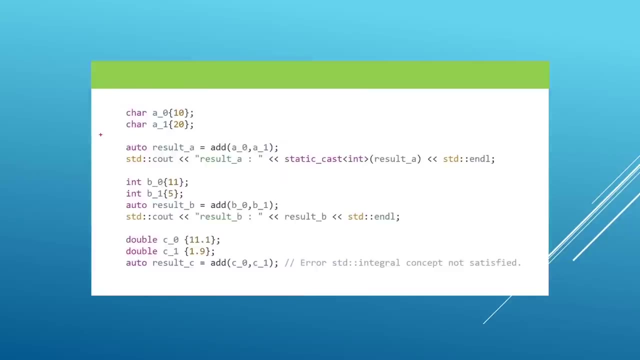 are going to get a compiler error. okay, once we have this concept set up, we can look at a piece of code that tries to use it and try to guess what is going to happen. here is a piece of code we would set up in the main function and try to call our function template. we have two variables of car. 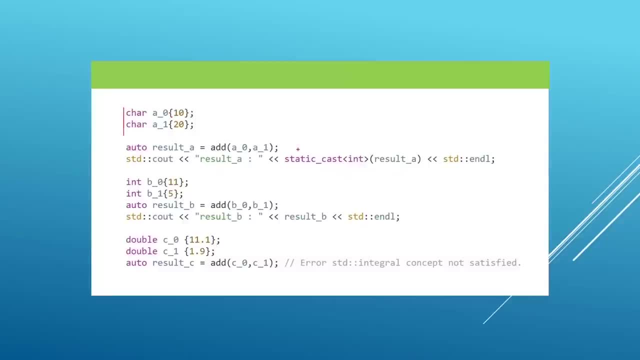 type. we know that car is an integral type. so if we issue a call like this, this call is going to work, the template instance is going to be generated and it's going to be called and give us the results that we can print here. this is right. on the second piece of code, here we have two variables. 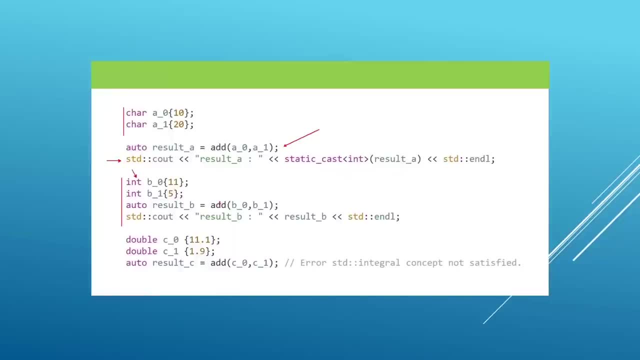 of type and we're going to call them. we're going to call our function template with and, and this is also an integral type. int is an integral type, so this is going to generate a function template with int, and this is also an integral type, so this is going to generate. 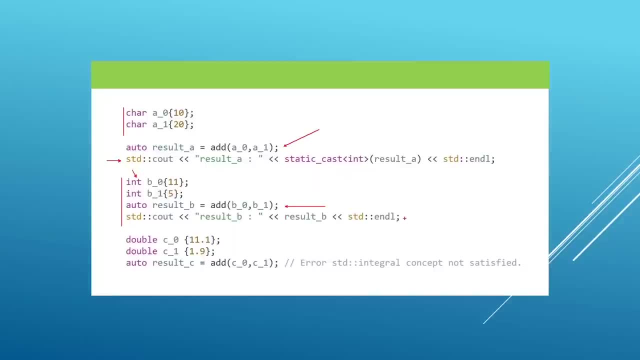 our function template instance and we're going to call it and get the results that we print here. and if we try to call our function template with double types, the concept is not going to be satisfied and we're going to get some kind of error and our function template instance is not. 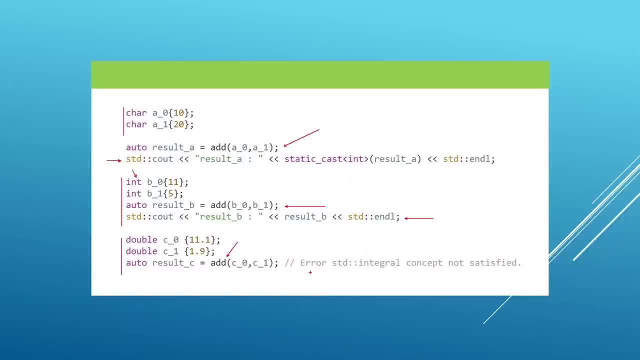 going to be generated. this is really how you can use concepts to force some rules on users of your function templates, if i can say it like that. we have been able to do something like this using type traits and static asserts in the last chapter, but concepts are much cleaner in that they are. 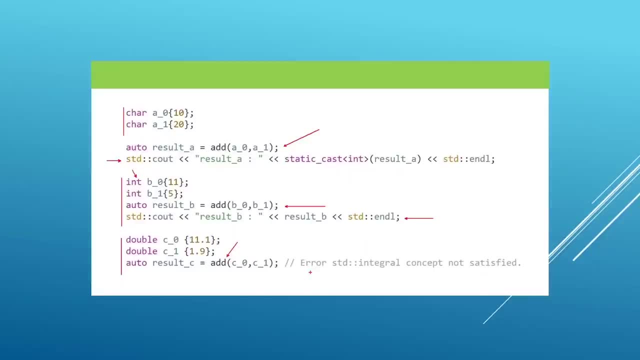 kind of built into the signature of your function. you don't have to go in the body of your function and set up static asserts. the function is already supporting concepts when you declare and define it, and this is really cool. okay, this is our first syntax we can use to set up. 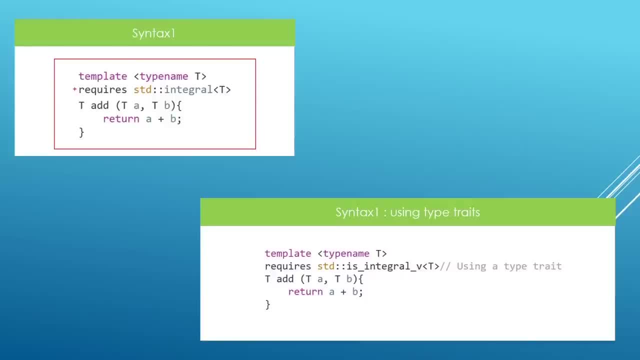 concepts for our function templates, using the requires clause after our template declaration and following that with whatever concept we want to enforce on our function template here. please note that you can also use type traits directly in the requires clause here and this is going to work and this really says that all you really have to put after the requires. 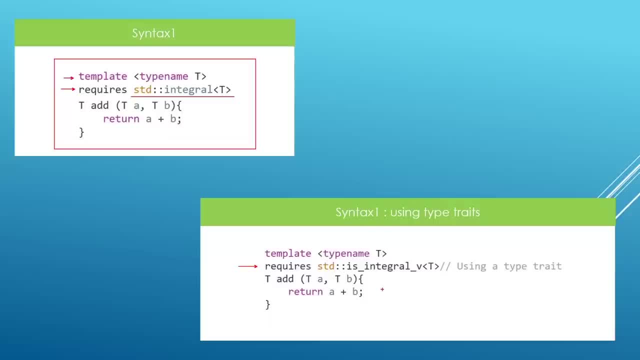 clause is an expression that can be evaluated at compile time but also results in a boolean value. once you satisfy these few requirements, you can really set up your concept however you want. you just have to be careful that the expression can be evaluated at compile time and that it evaluates to a boolean value, and when the 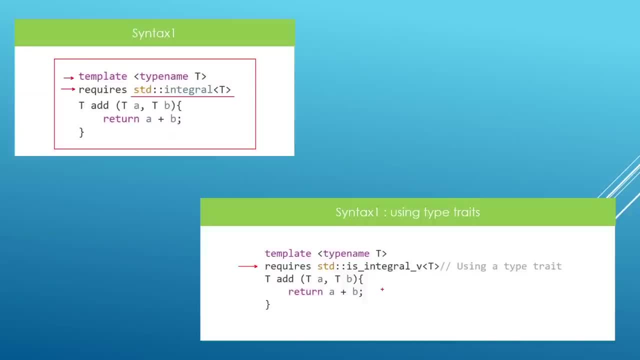 expression evaluates to true, the concept is going to succeed. if the expression evaluates to false, you're going to get a compiler error because the concept is not satisfied. this is how these things work. now that we have seen the first syntax, i think it is big time we looked at. 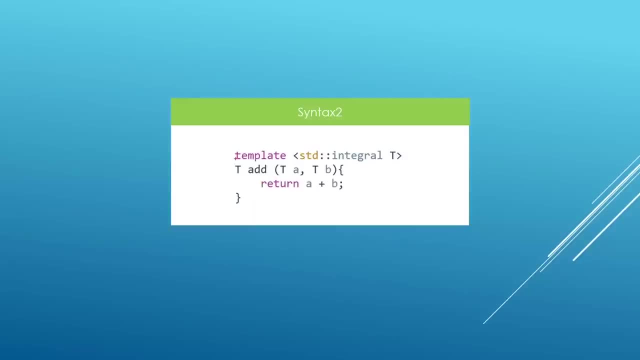 the second way you can set up concepts, and that's going to be in your template declaration. you're going to say template, put in your angle brackets and inside, instead of saying type name t, like we have been doing all along, you just specify your concept directly and say the template. 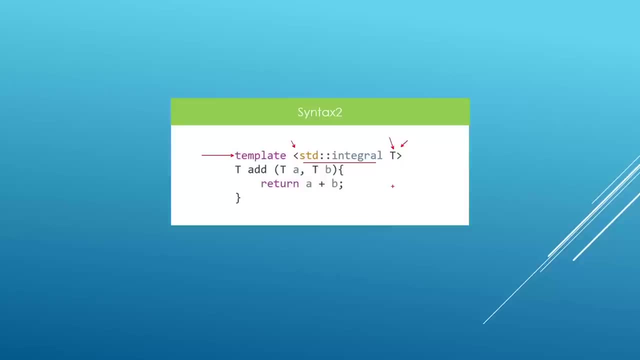 parameter like this. once you do this, this concept is going to be enforced on this function template here. this is just another syntax to really do the same thing. we also have a third syntax we can use, if we use auto, to set up our function templates, and the way this works is to just add: 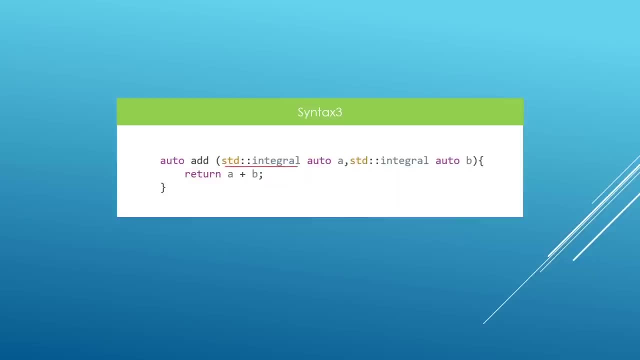 your concept in front of the auto keyword and once you do this, the compiler is going to enforce for the first parameter and the second parameter to this function to satisfy the integral concepts. so if you have to use auto to set up function templates, this is how you can use concepts to 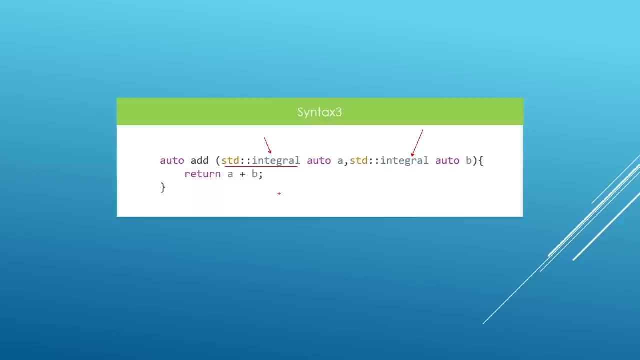 constrain ways in which people use your function. we still have another way. we can use concepts in z plus plus, and this is how you do it: you specify your template declaration, like we have been doing all along. you specify your function template, but after the parameter list, as we see here, you're going to put your requires close and you can put. 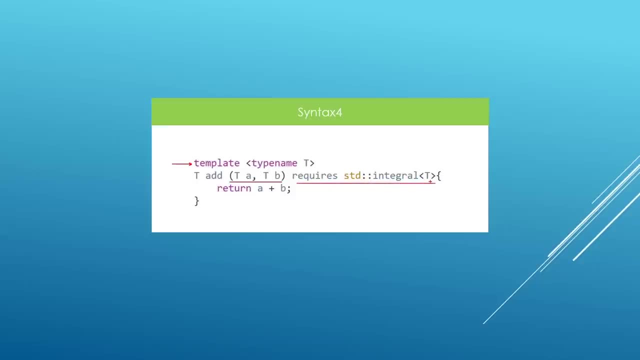 that in this place here and it is going to work. i realize these are many syntaxes to process for the first time, but some of these syntaxes are going to work better in some situations and they are there just to make it flexible for you to use concepts in your c plus plus code. okay, 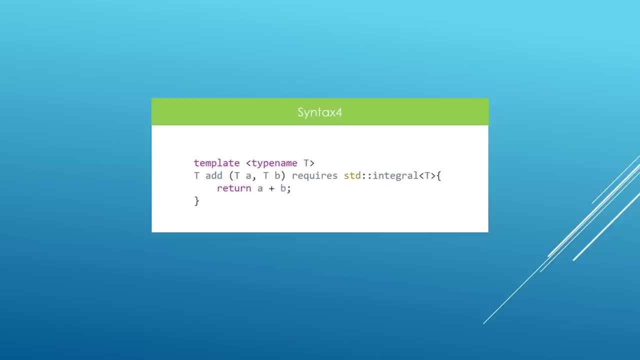 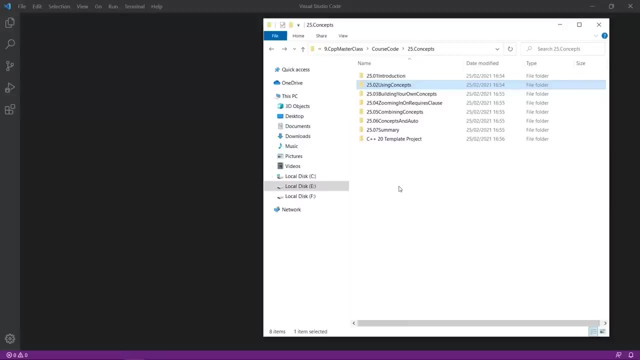 now that we have seen different ways we can set up concepts for our function templates, i think it is big time we headed over to visual studio code and tried them out. okay, here we are in our working folder. the current chapter is concepts. the current lecture is using concepts. 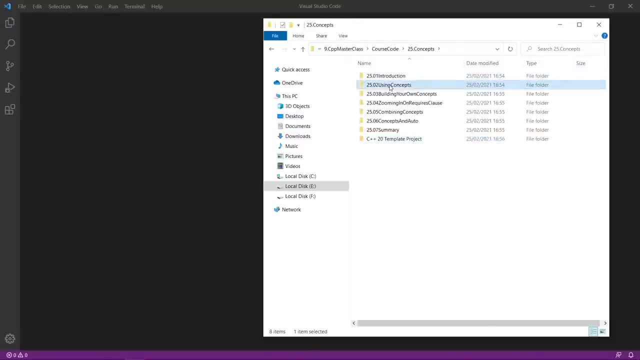 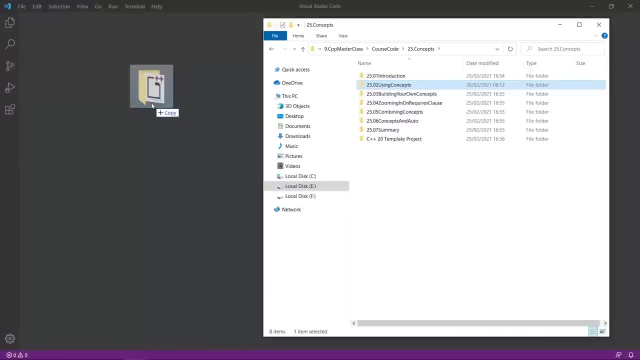 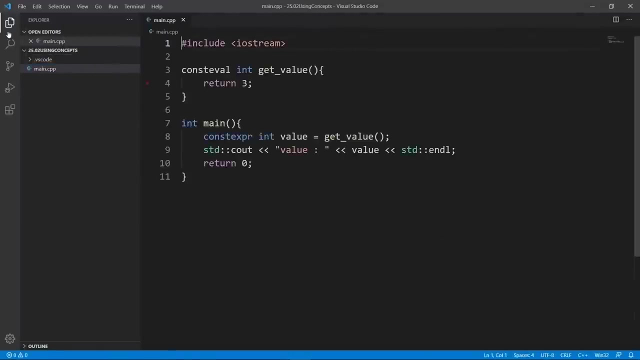 we're going to grab our template files, we are going to put them in place and we are going to this thing in visual studio code by dragging and dropping on top of visual studio code. here we do that. this is going to open our folder. we're going to open up our main cpp file and close the sidebar. 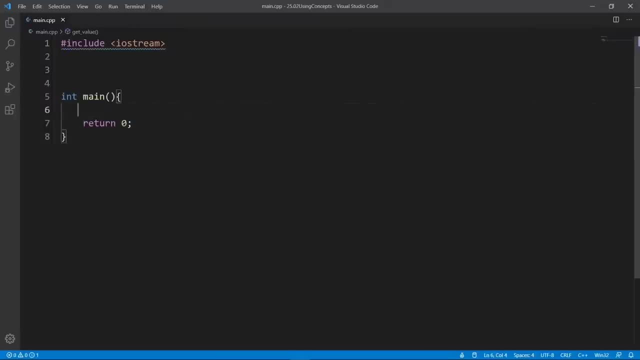 here and we're going to clean things up a little bit and we're going to set up our function template, which is going to add two numbers. we already know how to do that, so we're going to say template type name and it's going to have a template parameter of t. then we're going to set up the function like: 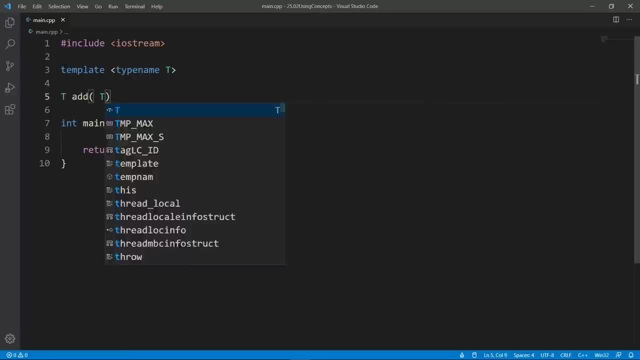 we have been doing all along. we're going to say add, we're going to say ta and tb and this is going to return the sum of a and b. once you have the function in, we can go in the main function and set up code that would call. 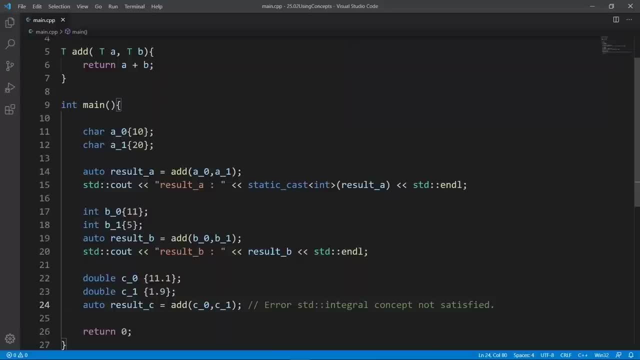 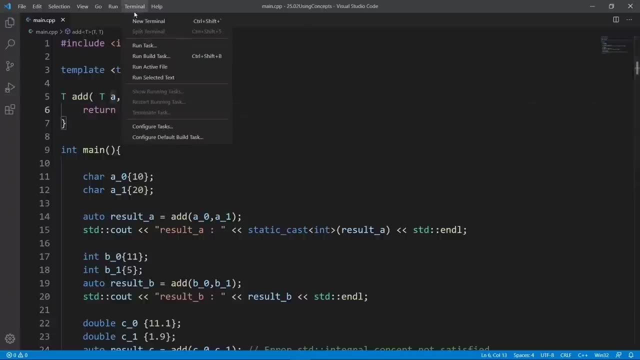 this function and if we try to compile this program, it is going to work now because we are not placing any constraints on this function template here. let's try to build with gcc, like we have been doing all along. you see, it is going to world, okay. you see, the world is going to be a. 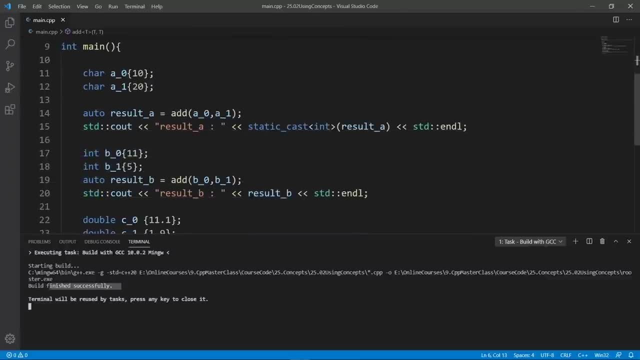 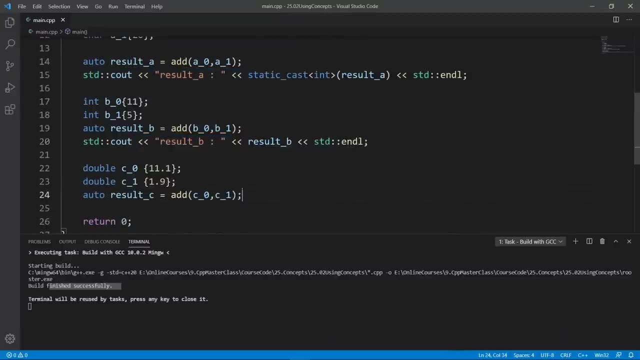 good world finished successfully and if we want, we can run this application and it is going to print result a, result b- let's take this out because we haven't done this yet- but it's not going to print result c. but if we want, we can really print it. it's going to work. so let's put that in and 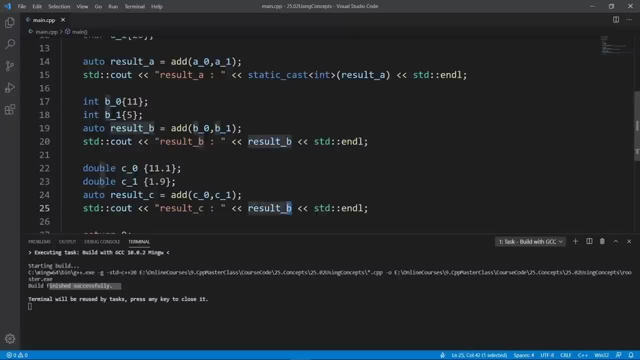 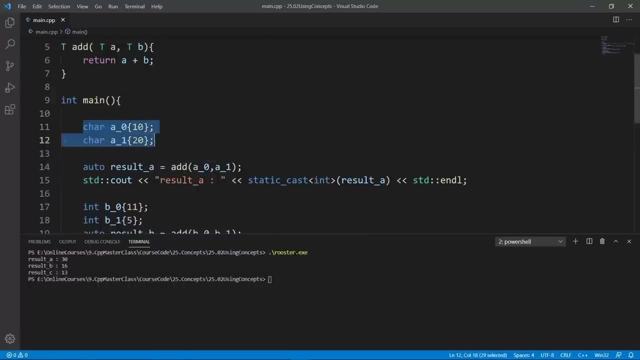 we're going to say result c and print result c here and weld again. let's weld now to take this into account. weld is good. we can bring up a terminal to try this out and we're going to print this out and we can clear and run rooster. now you see, result a is 30 because that's the sum of a and 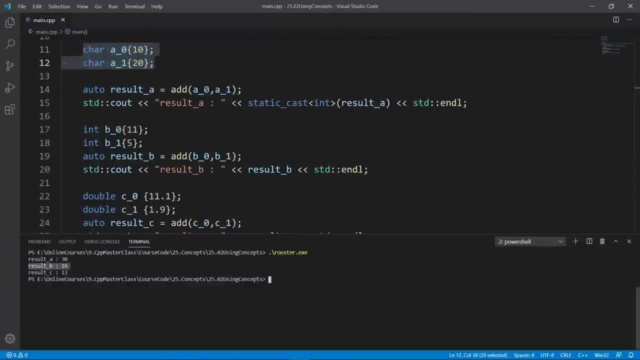 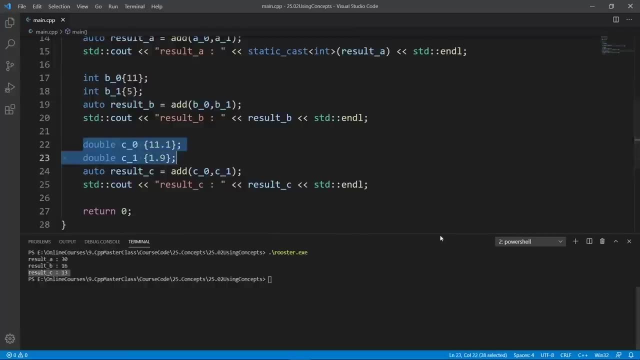 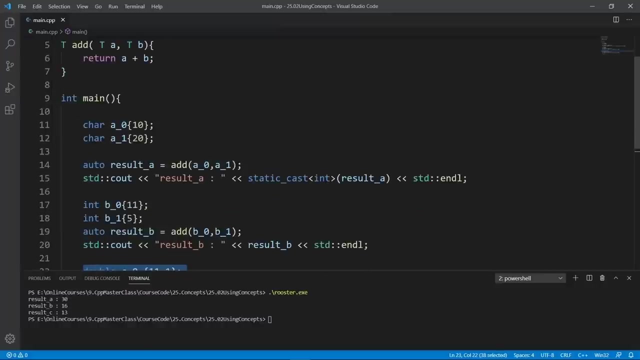 b here. result b should be 16, which is what we have. result c is 13, which is what we should get by adding these two double variables. now we wanted to constrain this function to only work if somebody passes integral types, and when we put that constraint in place, it is going to work if we add. 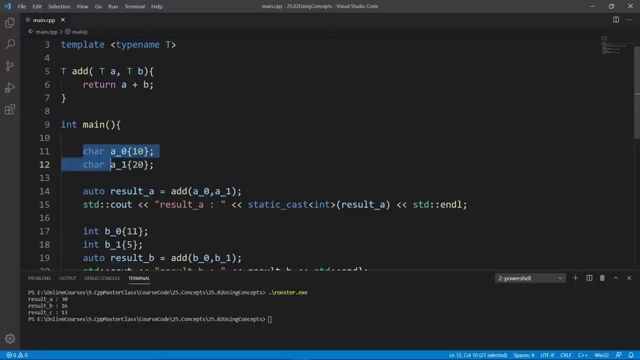 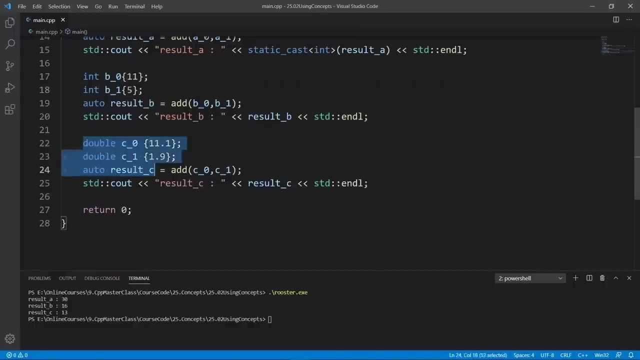 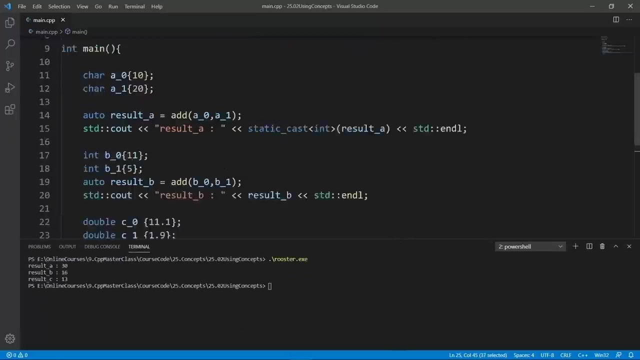 up two character variables because they are integral types. it's going to work if we add up two integer variables because they are integral types. but once we hit this guy here with double variables, we should get a compiler error because the constraint is not satisfied. let's do that. we're going to comment the double. 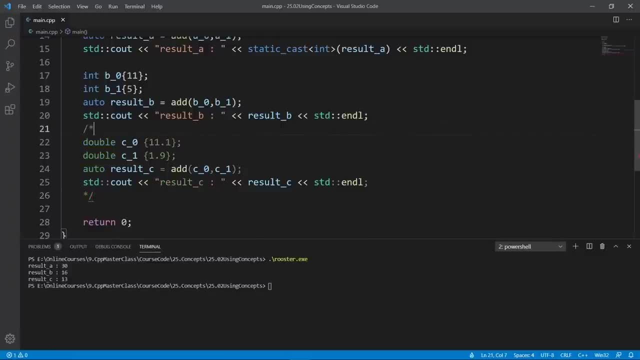 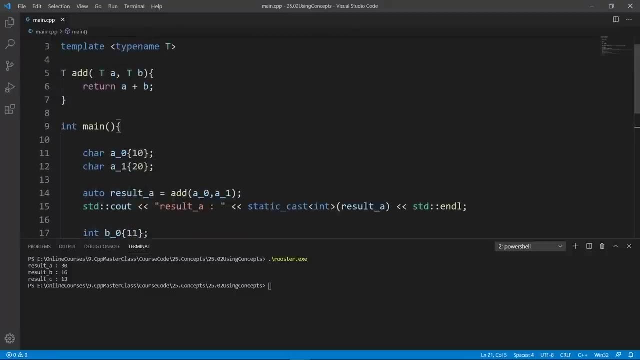 thing first, because we want to really isolate it and see it and see the compiler error that we get and we're going to add a constraint to our function template using concepts. okay, if you want to use concepts in c plus plus 20, the first thing you need to do 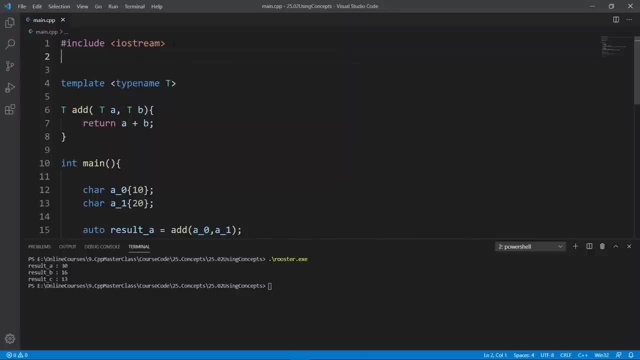 is to include the library that gives us access to concepts, and we're going to do that by saying: include concepts. this is easy now that we have this, and we're going to use the first syntax we saw in the slides and we're going to add the requires clause after the template declaration. 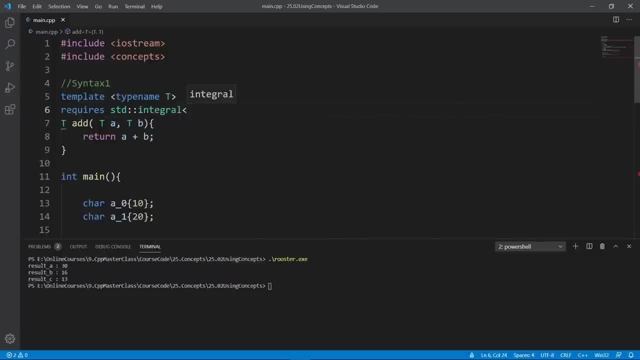 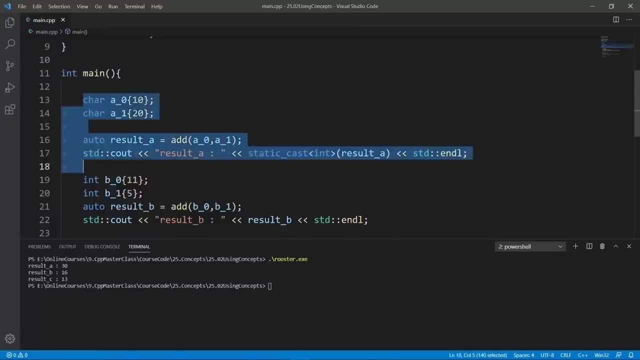 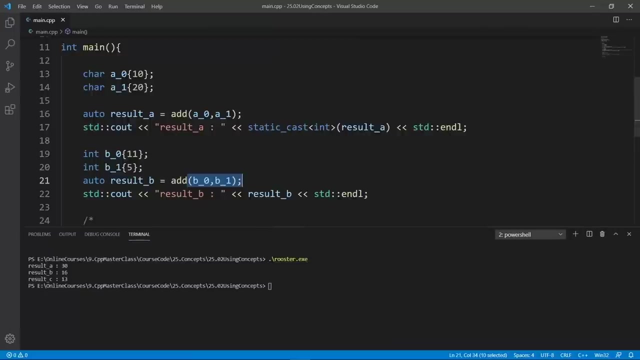 and we're going to say std integral and we're going to say the template parameter here. i think this is the syntax. okay, what if we собd this? all right, in the relentless Rust? assign whatever repairing is this and this one. okay, watch what happens. if we do this down in the code, we are calling the function with: 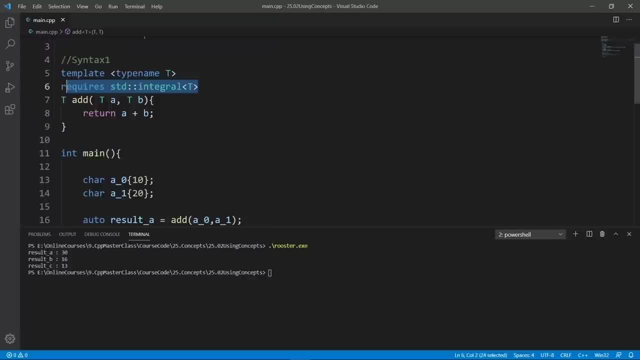 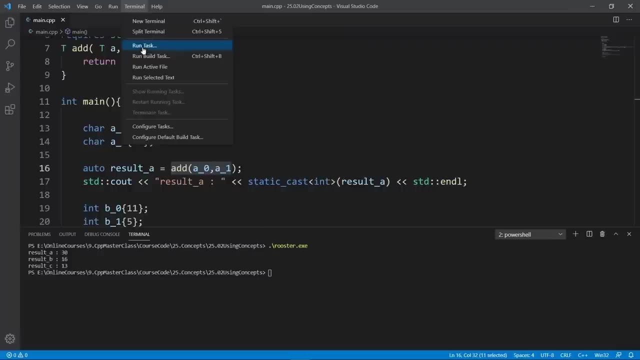 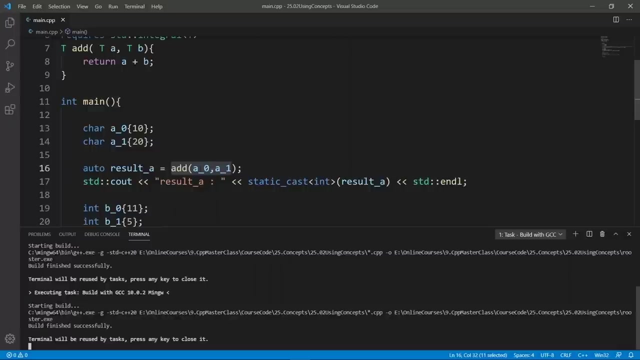 car types and integer types. so this is going to compile. fine, because the concept here is satisfied. this concept is going to enforce for the template parameters we call our function template with to be integral types. let's build and see if we, if we run our program, we should see results, a and result to be printed out. let's run the program. we. 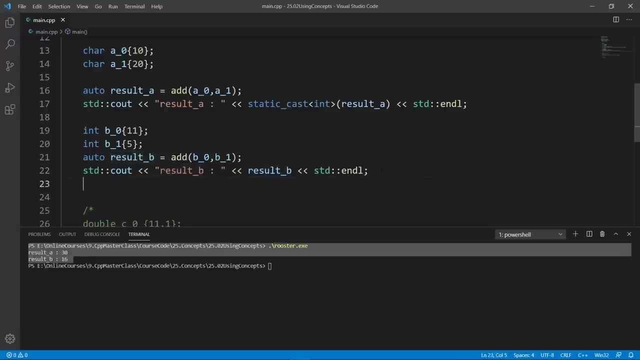 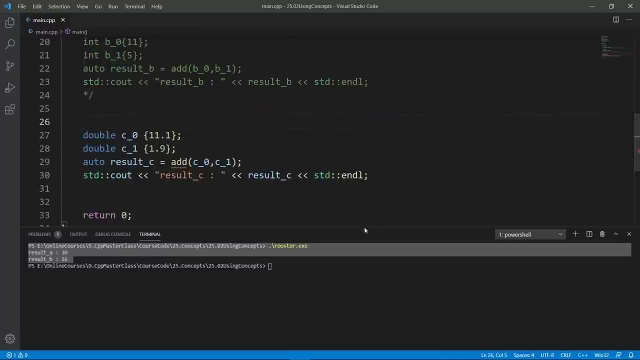 see our results here. now we're going to comment out the others and leave in the double example and we're going to uncomment that. and i want you to see the problem we get when we try to use our function template with double variables. here you see, visual studio code is already complaining it. 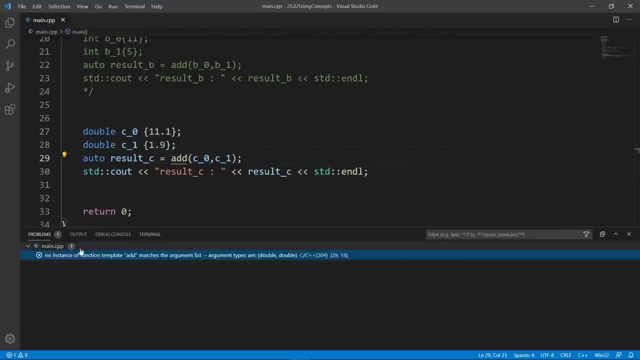 is saying there is something wrong. if we look at the problems tab it's going to say no instance of function template. ad matches the argument list. but this is really not descriptive enough. but the problem is our concept is not satisfied by calling our function template with double types. 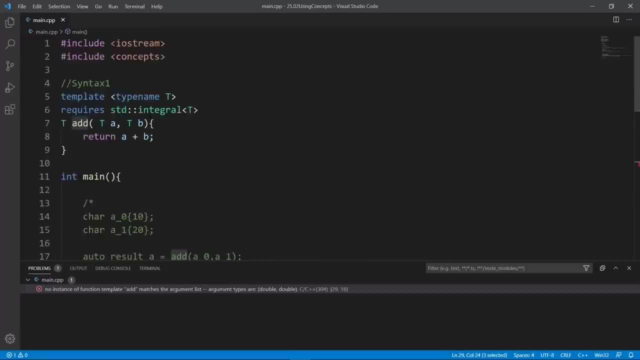 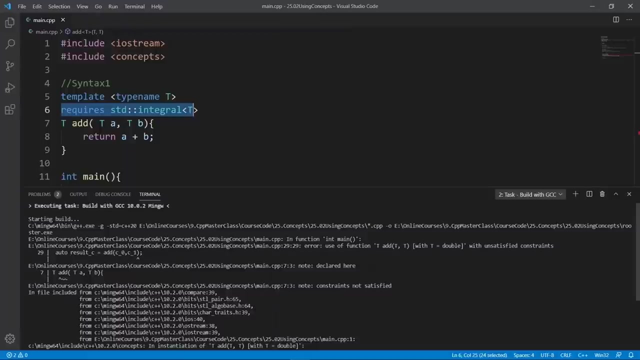 because we clearly say that we want the function to only be called with integral types. let's build our program, we're going to pass this through gcc and we're going to get a compiler error that says that some concept was unsatisfied. and we see, we see in function main use of function t add with double, with unsatisfied constraints. 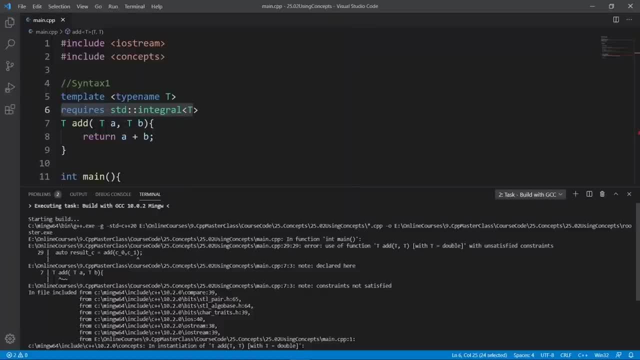 and this is really clear. when we see an error like this, we will go and look at the constraints that the function has and we're going to see if we satisfied those constraints by calling like we did in the main function here, and we will no that the function doesn't support non-integral types and we will fix this problem. this is really. 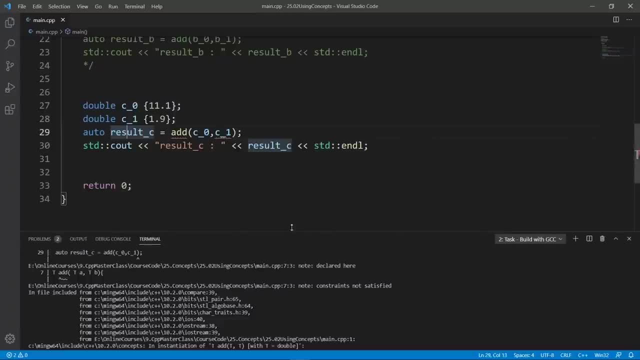 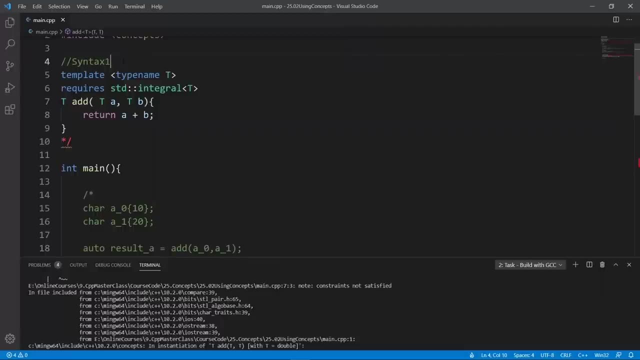 how concepts can help in writing. safer function templates. now that we have seen the first syntax, i think it is big time we looked at the other syntaxes. so let's do that. let's copy the code here, because we're going to be reusing this a couple of times and adapt it instead of typing. 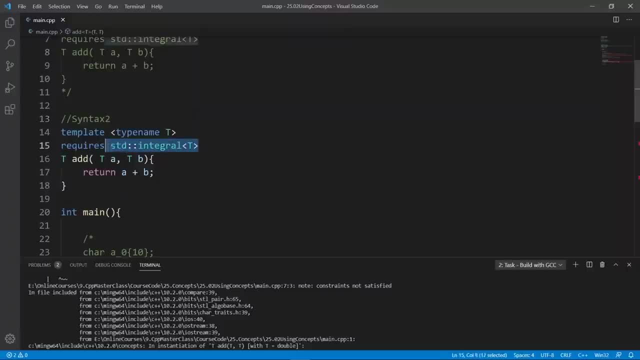 this entire thing. the second syntax involves getting rid of the requires close all together and just using the concept instead of type name here. so i'm going to say std integral and this is going to be enough. this is going to tell the compiler to enforce this concept for this function. 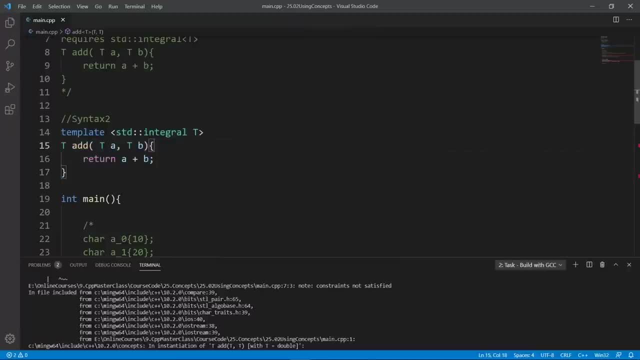 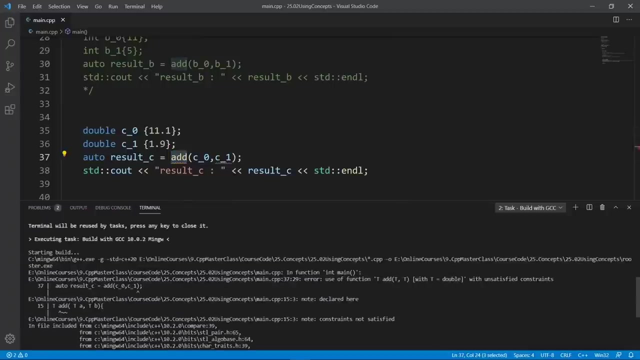 call for all the template parameters that go in the place of t here. i hope this makes sense now. if we go back, will you see that you still have our squiggly lines here? if we try to compile we will get the same compiler error- okay, and you see we have the same compiler error. function add t, called with unsatisfied constraints. 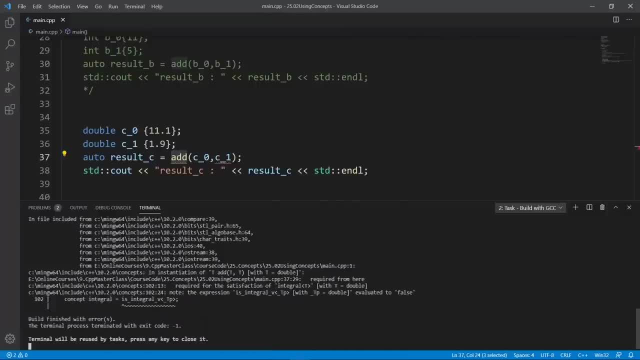 i think if you go down we're going to see even more stuff out of this. it's going to say: required the satisfaction of std integral with t, but now we are trying to call this with double, so this is really going to lead to a compiler error. so this is the second syntax and it is going to 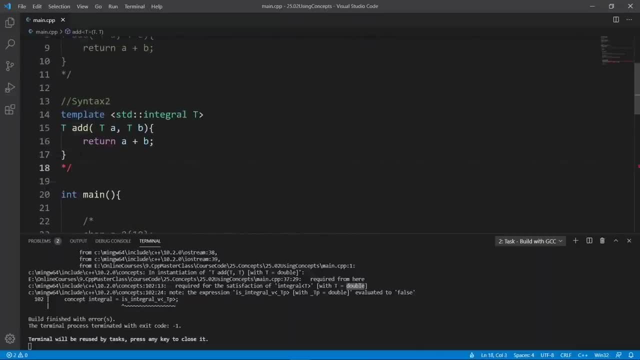 do the same thing. now that we have seen this, we also have a third way we can do this and that's through the auto mechanism. let's set up our function using auto. so we're going to say auto add, auto a and auto b. we have seen that we can do that in the last chapter and we're going to return. 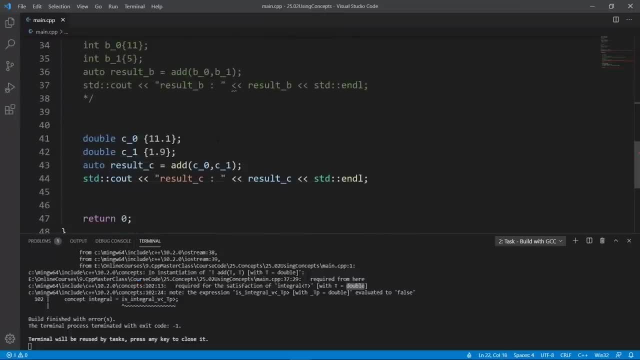 a and b, a plus b, i should say. if we do this, you see that the squiggly line goes away and we can add these things up and print the result. the return type is going to be deduced by the compiler automatically, but know that this is going to generate a function template behind. 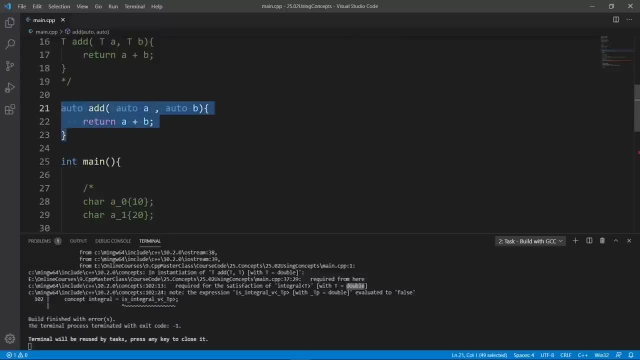 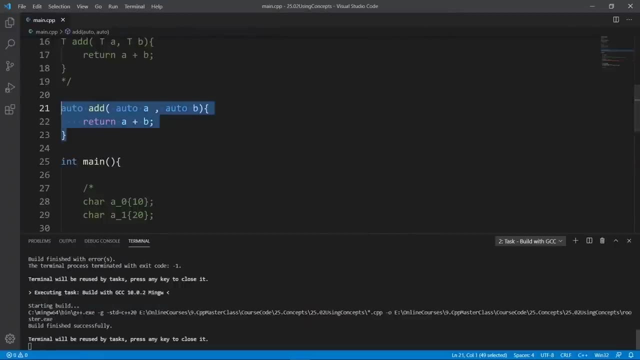 the scenes. this is just a nicer syntax. we have to use auto to set up functions that work for multiple times. let's build and see how gcc handles this. the world is good because we have no constraints here and if we run our program, it's going to work. it's going to give us 13 as the sum. 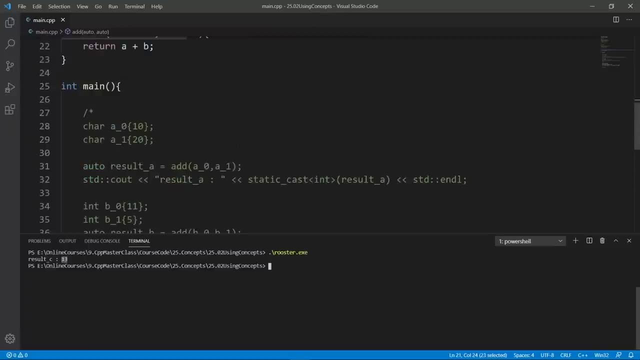 of 11.1 and 1.9. but we can also place constraints on this function here, and you do that by specifying your concept in front of the auto keyword here. so for example, we can say std integral and std integral for the second parameter here let's say that. and once we do this, if we go down, 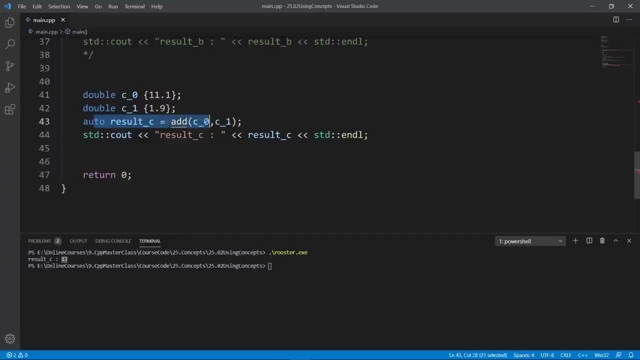 we should see our squiggly line on the call of the function here, because now the way we are calling this function is not valid. that's why we need to use it, because it's not valid. if we're going to function clearly says that it wants to be called only with arguments that satisfy this concept here. 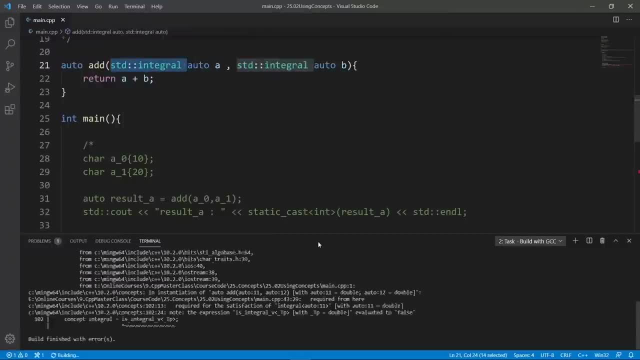 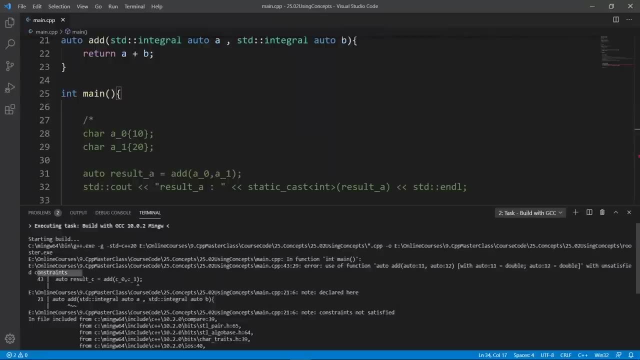 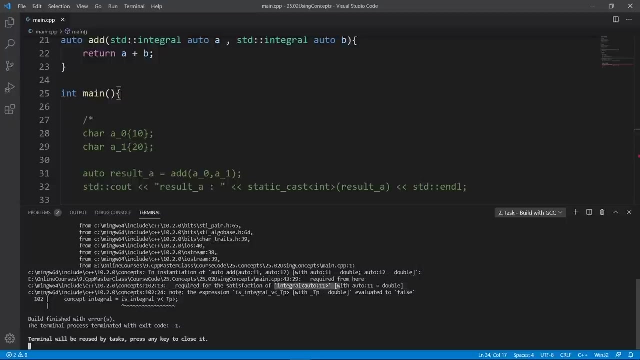 if we try to build again with gcc, we're going to get the same compiler error- let's do that- and it's going to say: use function with unsatisfied constraints- the same error. and if we go down we should see that it requires the integral concept to be satisfied here. so this is the 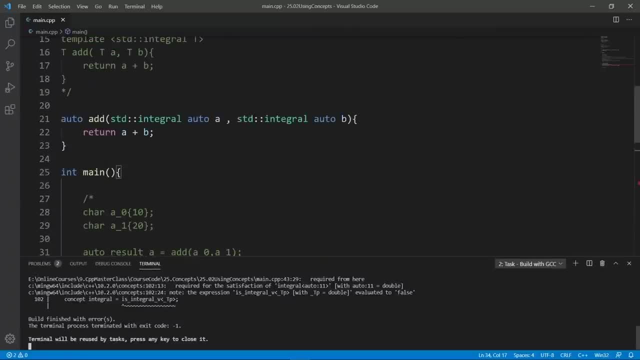 third syntax you can use. if you happen to be using the auto syntax for your function templates, let's comment this out, because we still have another syntax we need to learn about. this is going to be our syntax 3 and we're going to comment this out. and the last one involves just leaving in. 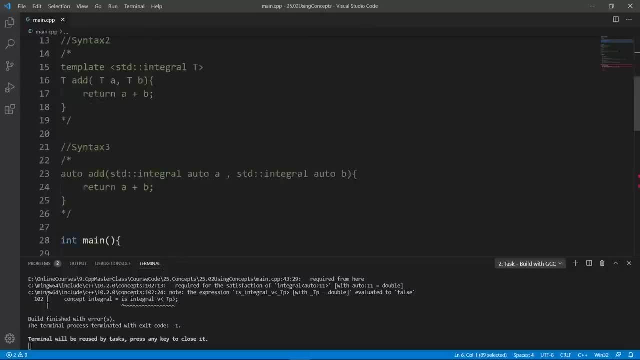 our function template. let's copy this because i don't want to type this again. we're going to go down and say syntax 4 and put in our function template. we're going to take this requires close. we're going to cut it out and we're going to put it after the function parameter list. 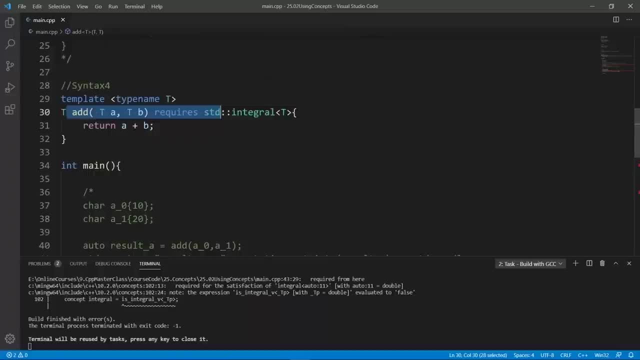 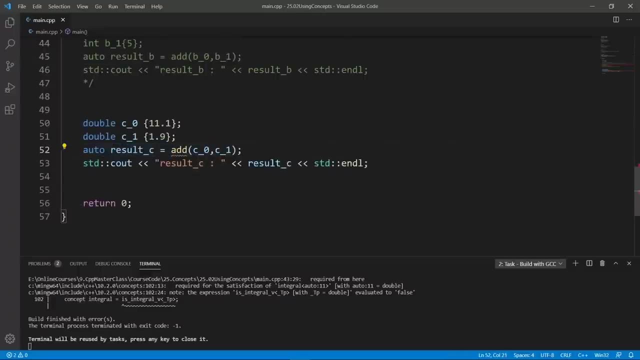 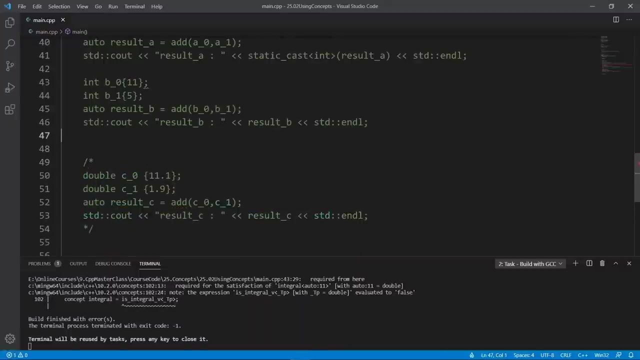 like this, and this is going to be valid c plus plus syntax to enforce a concept on your function template. if we go down, you see we have this wiggly line and i should prove that this works with other integral types here. let's just comment out the double line here, and and: 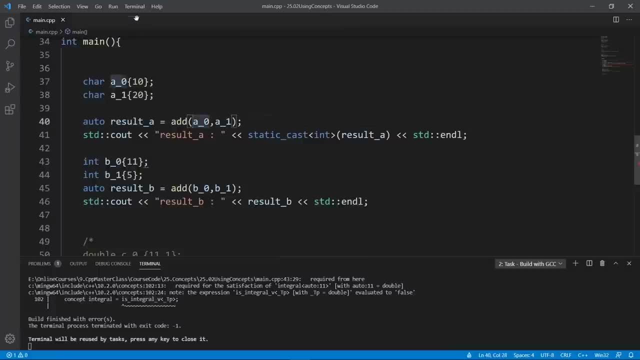 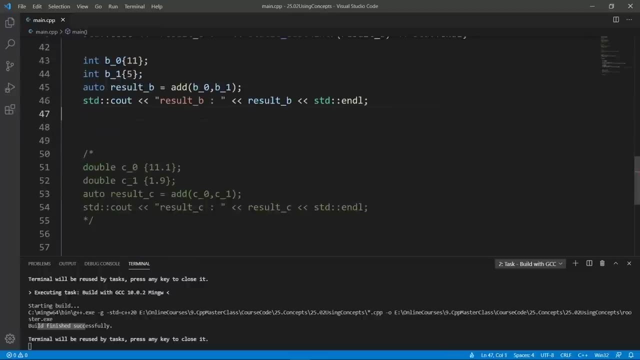 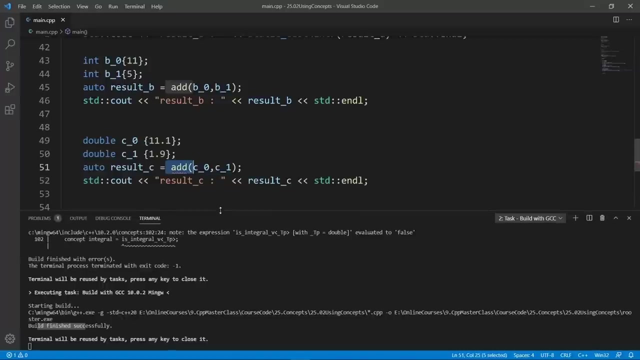 comment, the other we had for car and end. if we're trying to build this program now, it is going to be is going to world fine because the constraints are satisfied. but the moment we uncomment the calls with double types we're going to get a squiggly line, which is a good warning that we 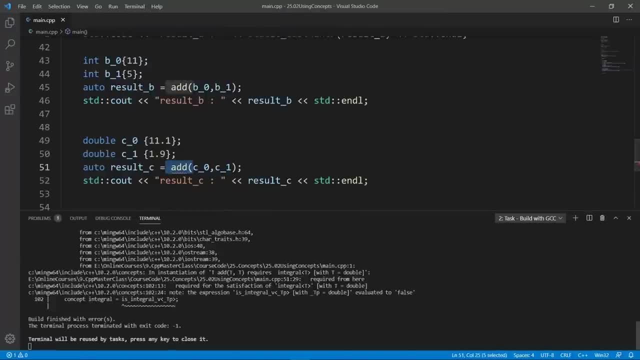 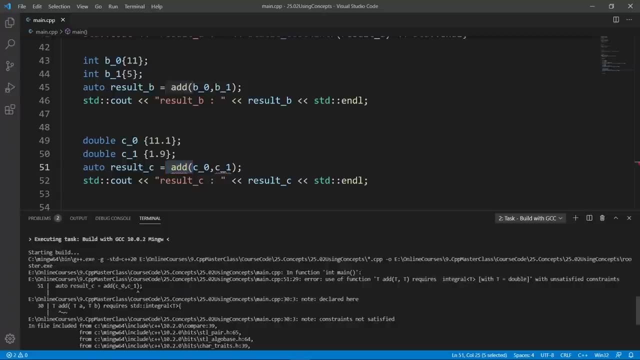 have a problem. but if we ignore the squiggly lines and just build with gcc, we're going to get the same compiler error and it's going to say that to call our function we need to satisfy the integral concept, for the arguments that we pass here and the double arguments we're passing in here are violating our concept. so we get. 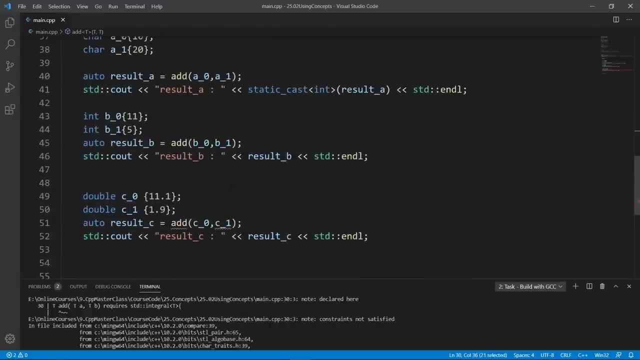 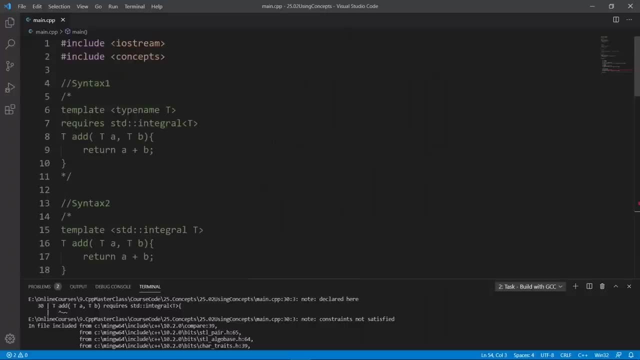 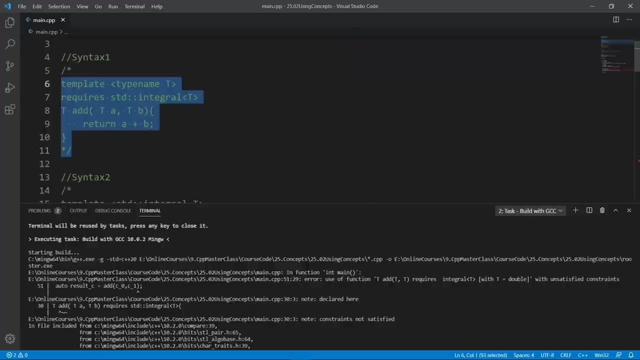 our compiler error. this is really how you can use concepts in c plus plus. i tried and came up with simple examples to show you different syntaxes you can use concepts with. and this is really it. try to get yourself familiar with these syntaxes and it's not going to be really hard to use. 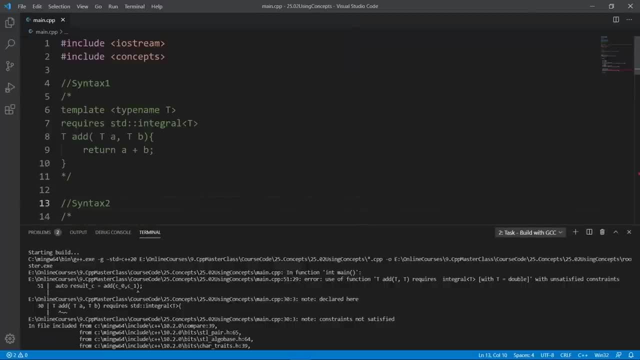 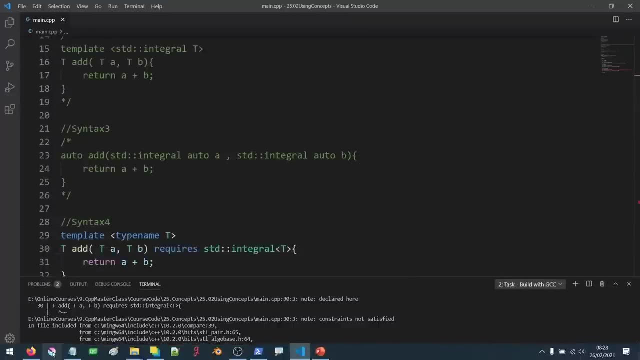 concepts in your c plus plus programs. okay, this is really all i had to share in terms of the syntaxes you can use with c plus plus 20 concepts. if you go to the documentation, you're going to have more information about this, but we're going to do a few more. 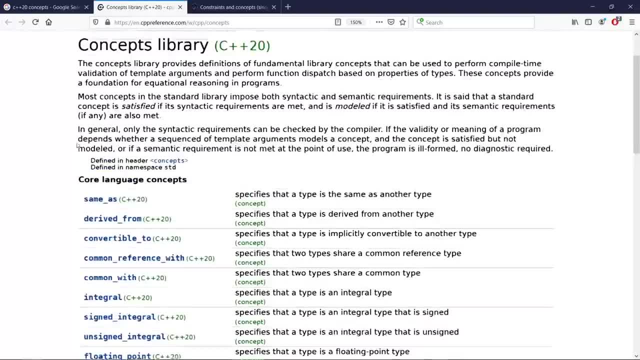 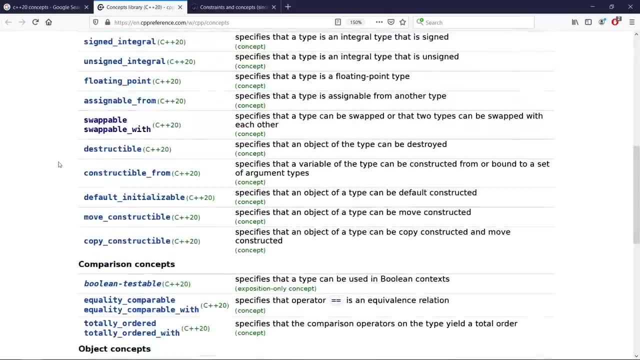 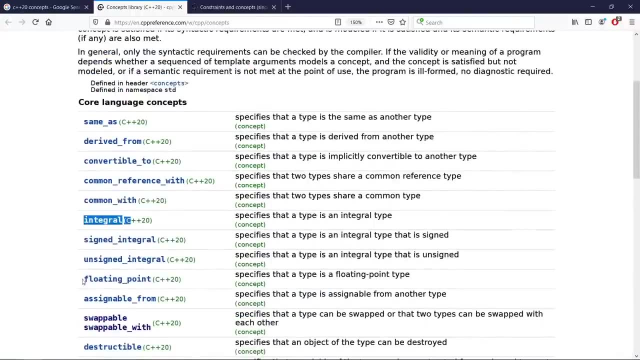 lectures to really drive these things home. for now, you can come to cpp reference here and see more concepts that you can use. we have a lot of this and we can really use this to tune our function templates however we want. okay, for example, you see our integral concept. you see a. 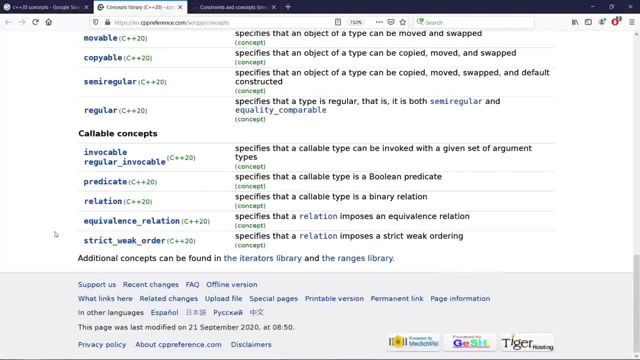 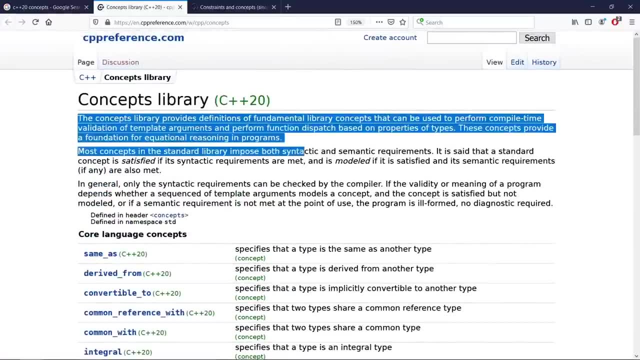 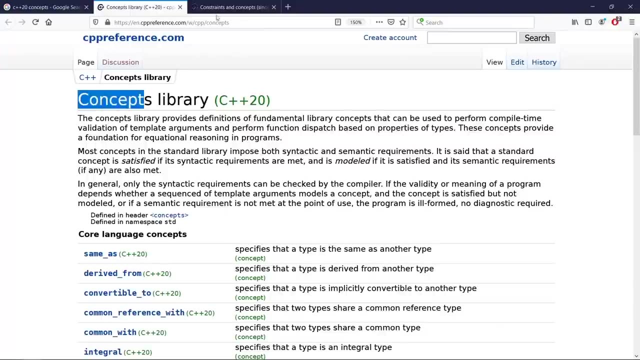 point concepts, and there are even more that are usable with classes. but we haven't learned about classes yet and we will do that starting in the next chapter. but now i just want you to be familiar with concepts that were introduced in c plus plus 20.. and here is another piece of documentation. 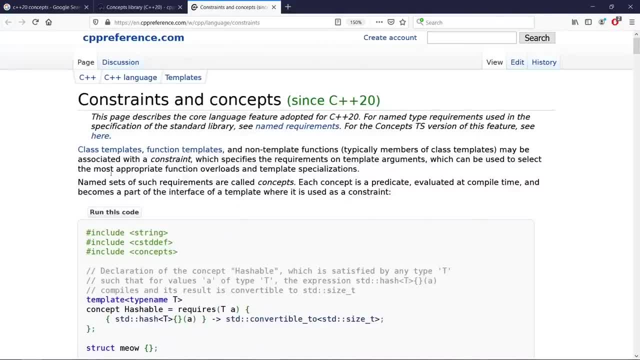 you can look at just to complement what we are talking about in this chapter, but i wouldn't recommend reading this just yet because it's just going to confuse you. there is a lot of things we still need to learn to really be able to understand this, so try to go through this. 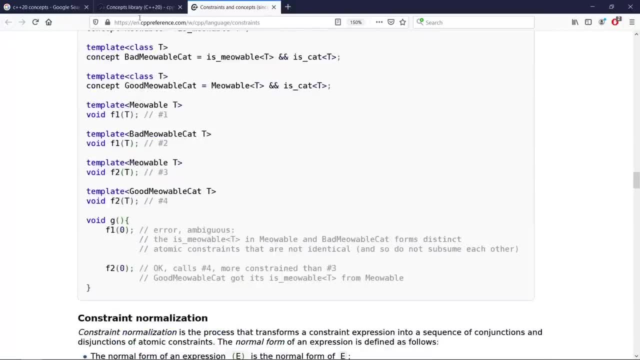 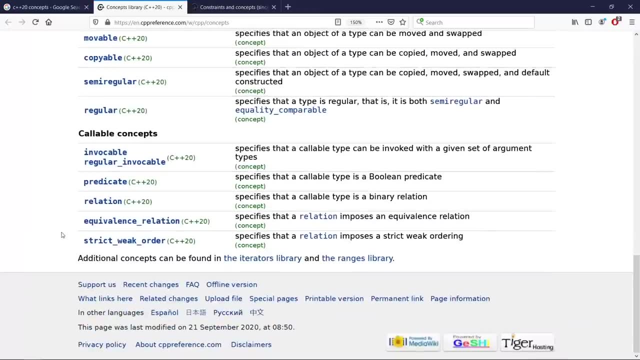 chapter and i am going to try and break this down in ways that you can understand this. the main message is that there are more concepts here. you can try in your c++ code if it makes sense for the problem you are trying to solve with c plus plus. we are going to stop here in this lecture. in the 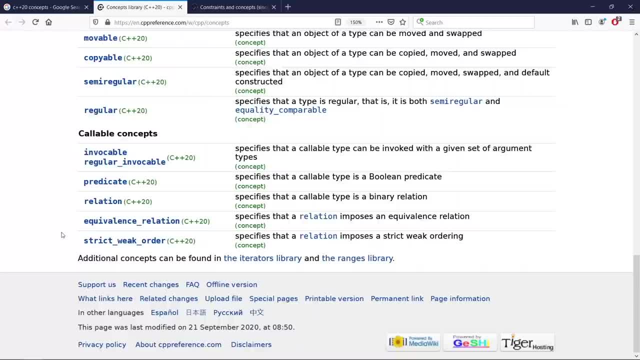 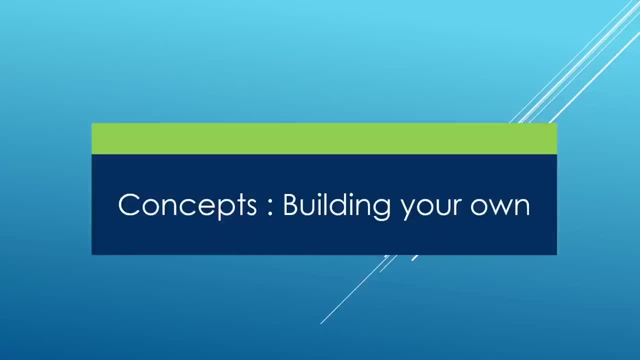 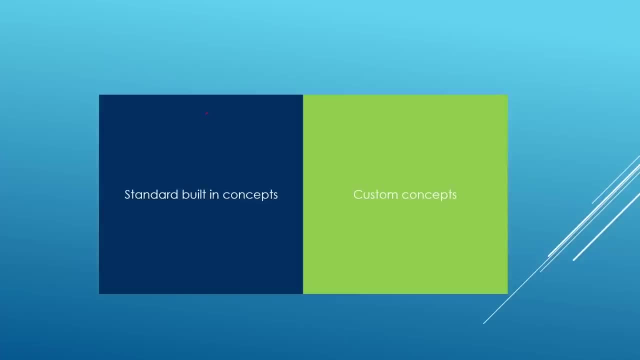 next one we're going to show you how you can set up your own concepts in c plus plus. go ahead and read me there. in this lecture we're going to see how you can build your own concepts, and this is going to bring us into the second part of concepts we can use in c plus plus. in the last lecture we 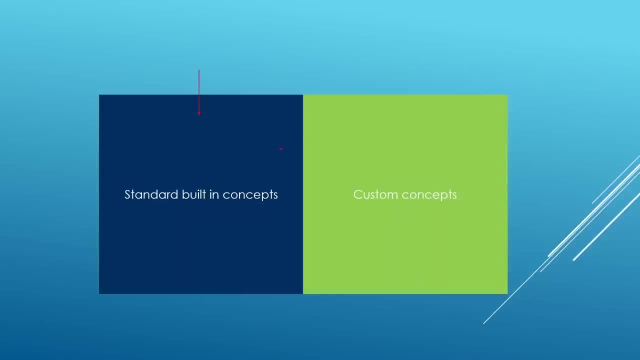 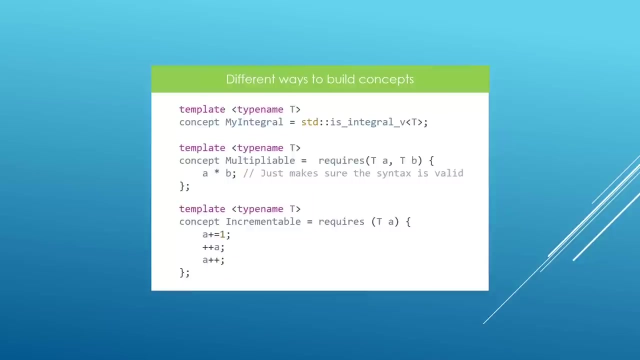 used the concepts from the standard library that are built into the c++ programming language, starting in c plus plus 20.. in this one, we're going to be building our own concepts and, without waiting anymore, let's see how you can do that, and this is the syntax you can use to do that. 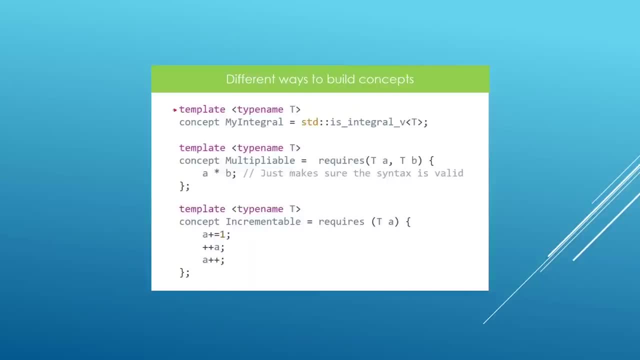 and it is really simple the way you do that. you say a template declaration specifying the template parameter you want to constrain, and then you say concept. you say the keyword concept, you give your concept name, you put the equal sign after that and then you're going to specify the requirements for. 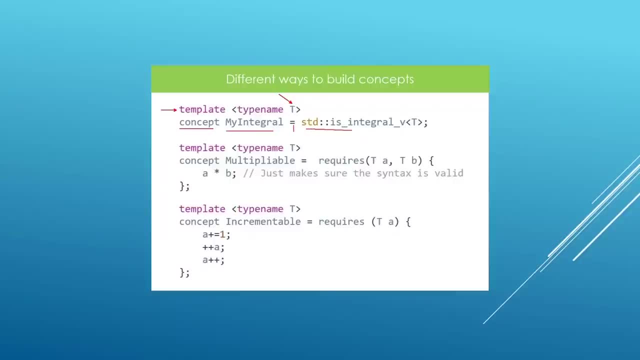 your concept. so, for example, here we are using a type trait to specify that this type trait is going to determine what works for this concept here, and what this is going to do is to enforce for our template parameter to only be integral. if it's not integral, we're going to get a compiler. 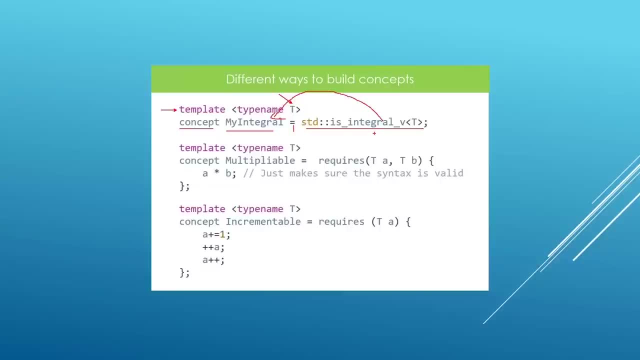 error. and one thing i should tell you is that the std integral concept is exactly built like this in the c++ standard library. this is really cool. so if you want to set up your own concept and you want to do that using type traits, you can do that like this and it is going to enforce. 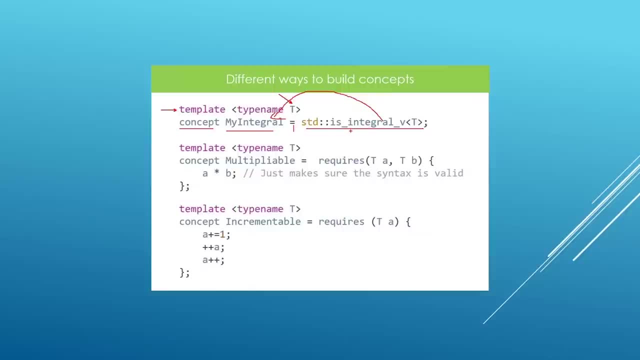 you can do that like this and it is going to enforce. you can do that like this and it is going to enforce for your template parameters to satisfy that type trait. or, to be exact, the concept is going to be satisfied when the type trait evaluates to true. if the type trait evaluates to false at compile time. 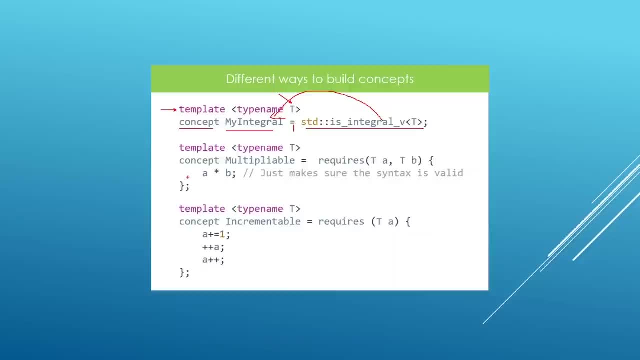 the concept is not going to be satisfied. that's another way to look at that. down here we have another syntax we can use if we have multiple statements in our concept. all you have to do is specify the concept keyword, you give it a name, and then you give it a name, and then you give it a. 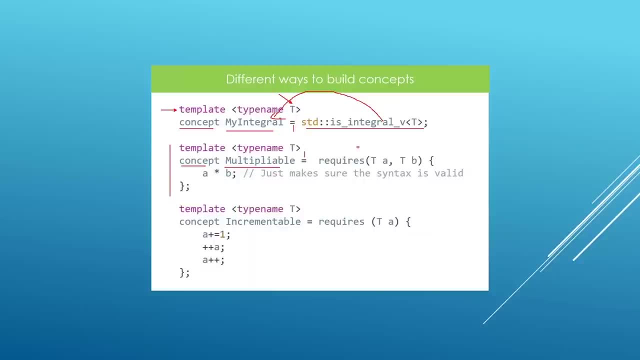 name. and then you give it a name, you put the equal sign and then you add a requires close. the requires close is going to specify the template parameters for which you want to enforce your concept. and then you're going to put a pair of curly braces and inside that you're going to 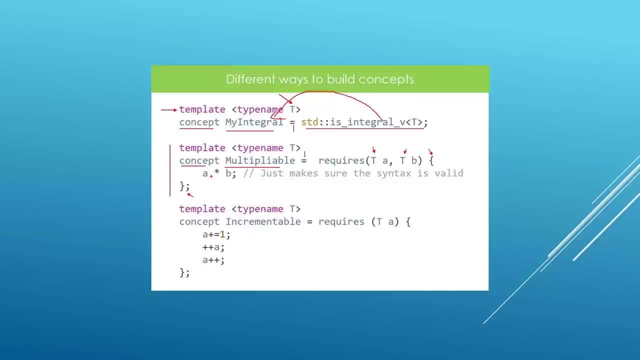 specify the syntax you want your concept to satisfy. for example, here we want for the two parameters to be supporting the multiplication operator. if this multiplication operator is going to be supporting the multiplication operator is not supported for the template parameters that we pass, the concept is going to fail. and again i should emphasize that this doesn't check for the 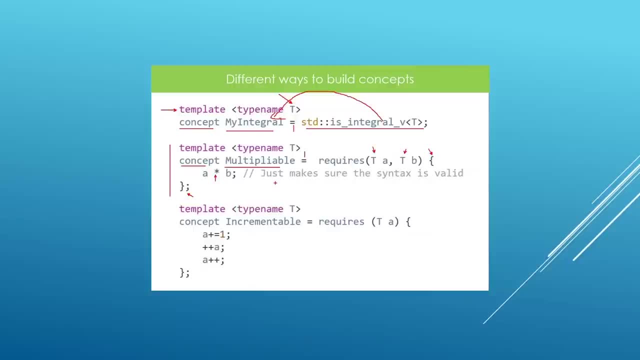 value of a multiplied by b. it's just going to enforce for the syntax to be supported. so, for example, if you call a function template with this concept and you try to pass in integers, it's going to work because you can multiply integers. but if you pass two strings, this is going to fail because 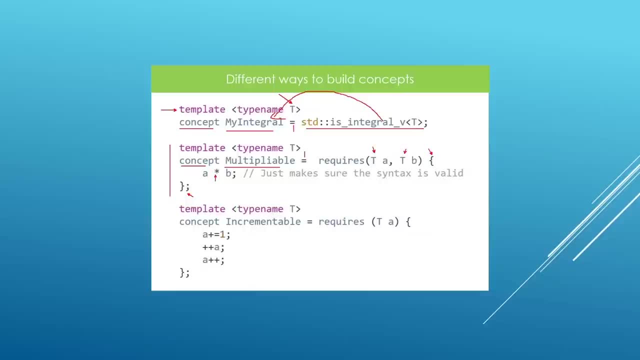 it doesn't really make sense to multiply strings. okay, this is the syntax. now we only have one statement to enforce inside, but if you want, you can even put more statements if you go down here. we have another example called incrementable. this is going to require for the template parameter to 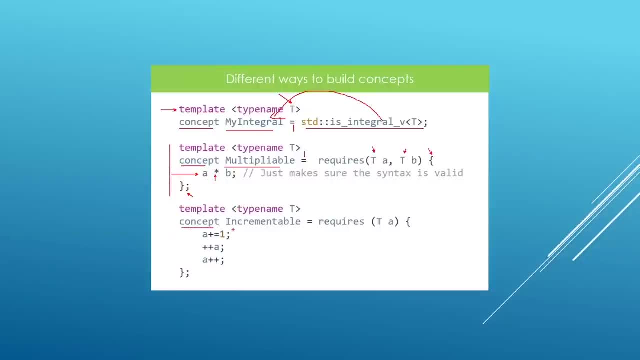 be incrementable. we specify the concept keyword, we say the concept name, we put in our equal sign and then we say requires: we put on template parameter and put in our requirements for any template parameter that is using this concept. the syntax here must make sense, so you: 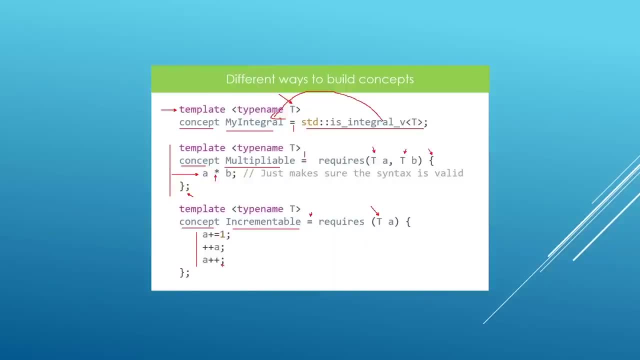 must be able to take the value that you get from here and, for example, say i plus equals one. this is going to be valid syntax. you're going to say plus plus a and plus plus b. all these are going to be valid c plus plus syntaxes for the template parameter that you try to call this function. 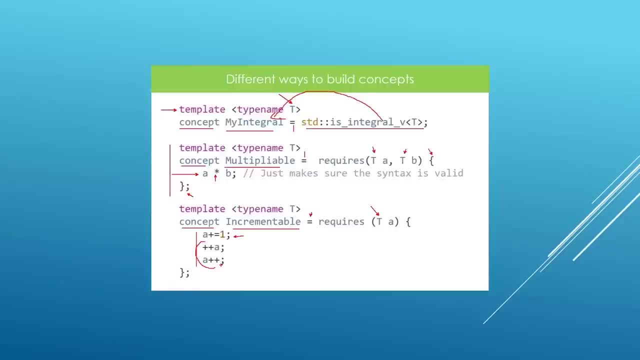 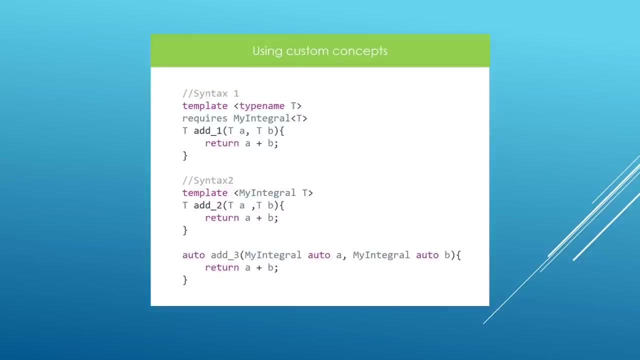 template with, and if this doesn't work, you're going to get a compiler error because your template argument isn't really satisfying this concept. so this is really how you can set up your own concepts in c plus plus. once you have your own concepts set up, you can use them like we have been. 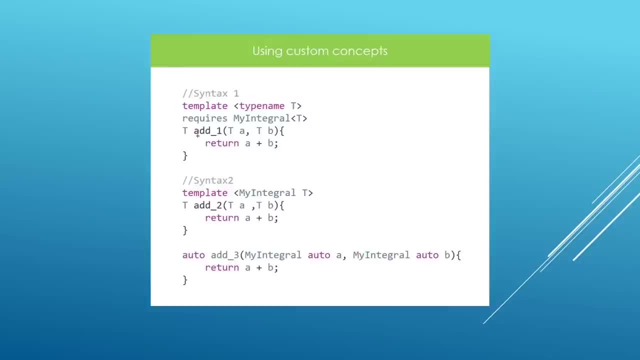 using the other concepts from the c plus plus standard library. for example, we can use syntax one to put a requires clause and say that we want to satisfy our own concept with this particular syntax. you will have to put in these angle brackets template parameter inside. this is the syntax you have to use. you can also use syntax 2 and specify: 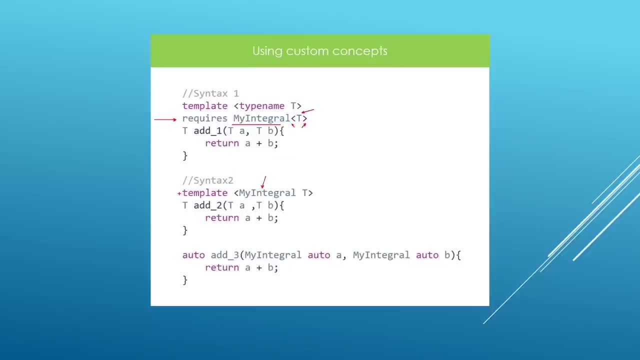 my integral directly in this angle brackets in your template declaration, and this is also going to work. we can even use this with the auto syntax for our function template. it is going to work. okay, now that you have seen this, i think it is time we headed over to visual studio code and play. 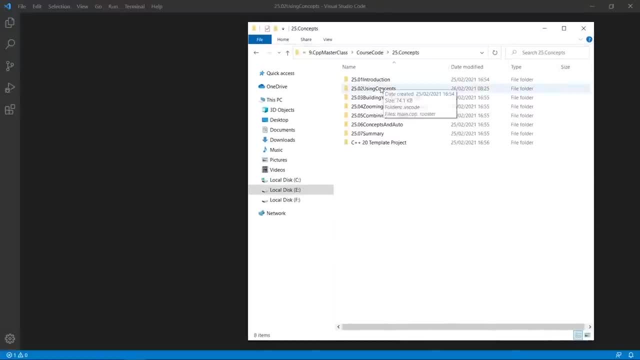 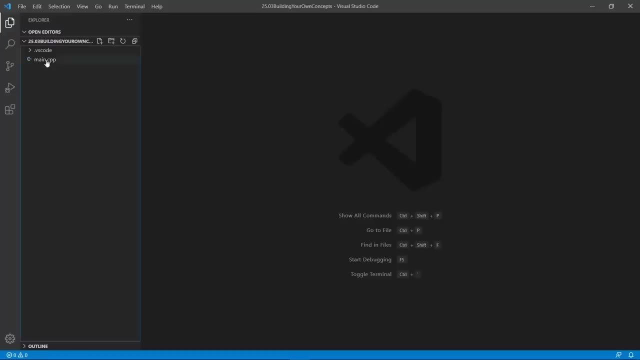 with this a little more. okay, here we are in our working folder. the current project is building your concepts. we're going to grab our template files, like we always do, and we're going to put them in place and we're going to open this thing in visual studio code. let's do that. we have our project open. 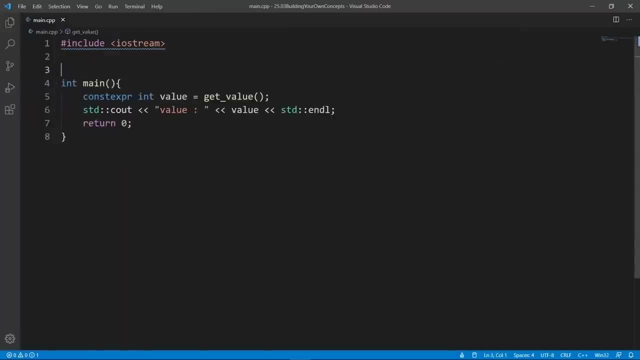 here or folder. i should say we're going to clean this up a little bit and we're going to include our concepts library and we wanted to set up our own concept. the first syntax we're going to see is by using type traits and we're going to say template, type name t and we're going to 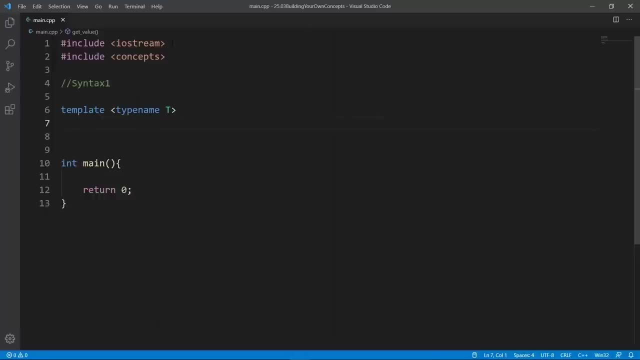 say this concept we want this template parameter to satisfy. we're going to say concept and we're going to say my integral, which is going to be the name of our concept. we're going to put an equal sign and then we're going to say std integral v and specify that we want this type trait to be. 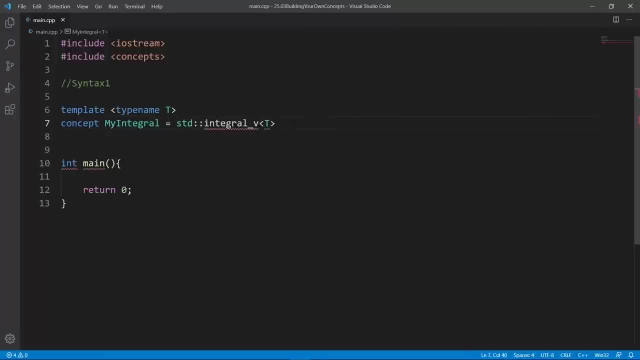 satisfied for this concept here and after this, we need to put in our semicolon- and i think we need to include the type traits library, because we're going to need to include the type traits library we are using- that we should say std is integral. so sorry for this and this is going to work now. 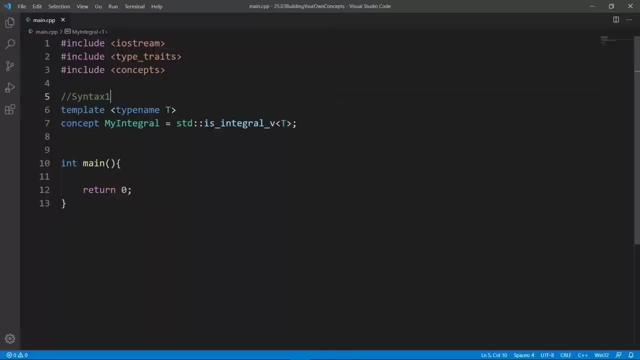 okay, now that we have the concept set up, we can use it like we have been using other concepts. for example, we can set up a function which is going to add up two numbers and it is going to use this concept. here we have multiple syntaxes we can use, so let's go down and try this out. we're. 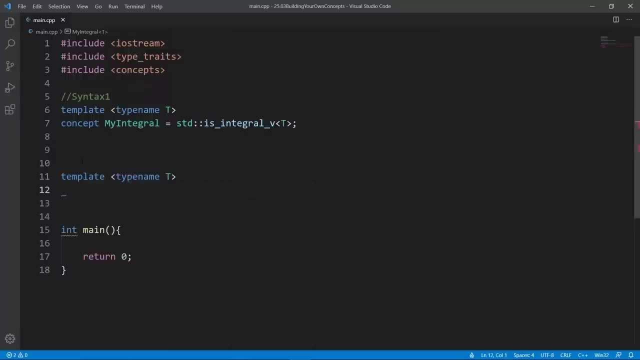 going to say template and say type name, team, and we're going to require this concept to be satisfied for our function template. we saw that we could use the requires close here and say my integral and say the template parameter. we want to enforce this on and after this we're. 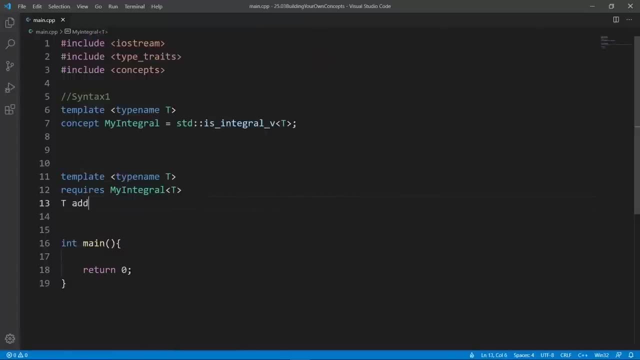 going to just put in our function template. we're going to say add what we have been doing all along in the last lecture. we're going to say ta and tb and we're going to return a plus b. now this function is going to support our concept. let's go down and set up two variables. we're going to say: 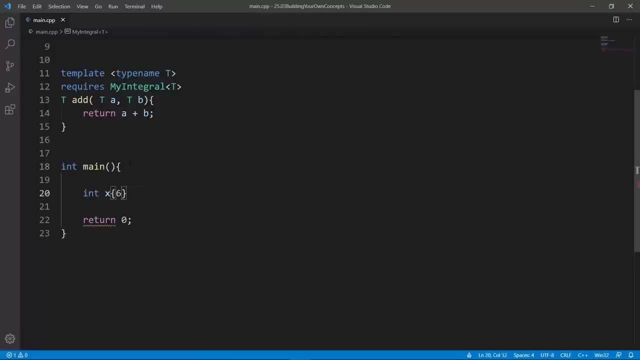 int x and we're going to say 6, for example, and into y, and we're going to make this a 7, why not? and we're going to say: add x and y. once we do this, you see that we have no problem, because the concept is satisfied for the arguments that we are passing in here. the concept is satisfied. 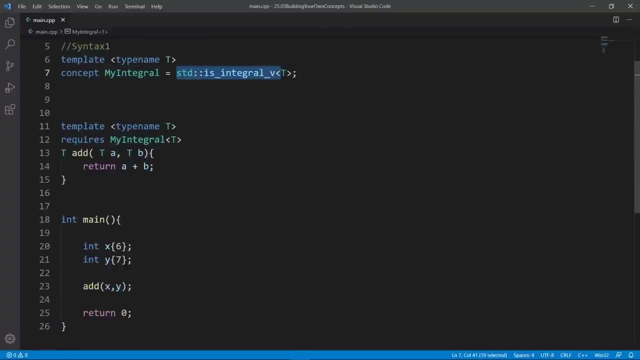 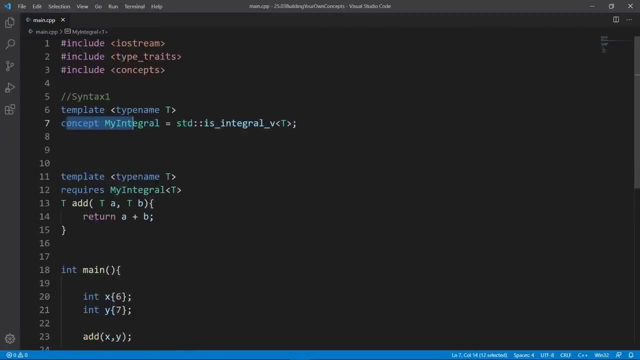 because the type trait here is going to return true for this type here, because it is an integral type. when the type trait returns true, then the concept is going to be satisfied. fine, if the type trait returns false, the concept is going to fail. let's try and bolt and really. 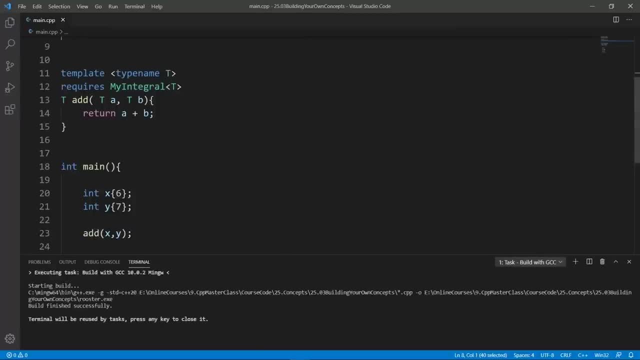 drive this home. you see that the world is good, our function is working. so the function template instance for this call here is going to be successfully generated and we're going to call it when the program runs. now let's change the type of these guys to double and try to violate. 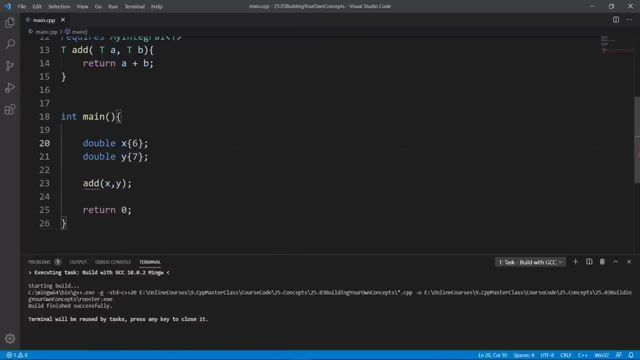 our concept and make it fail once we do this. you see, the call here has a squiggly line and a visual studio code is not going to say that. it is a concept problem, which is a shame, but we can still run this through the compiler and the compiler is going to tell us what is wrong. 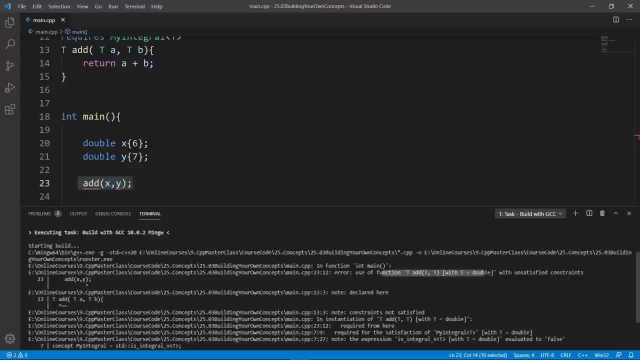 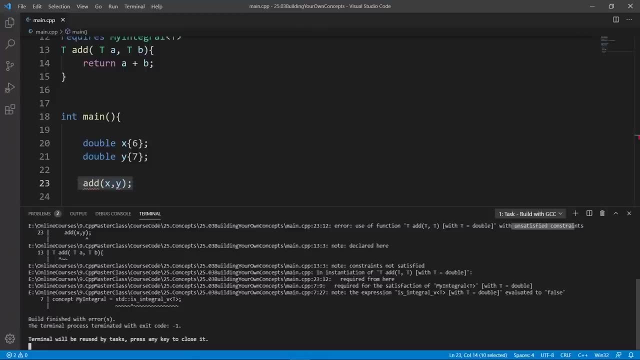 so it's going to say use of function add with unsatisfied constraints and if we go down we're going to see the exact constraints we violated and we're going to say required for the satisfaction of my integral with t. we are calling this with double and double is going. 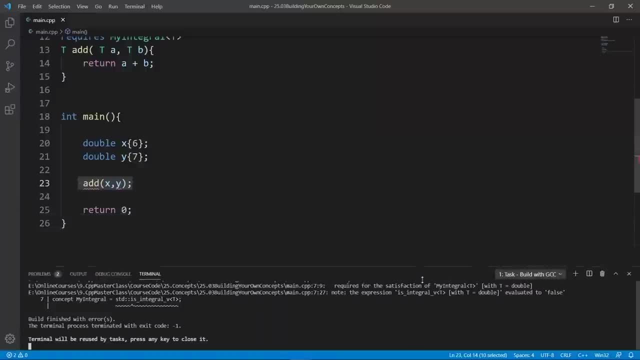 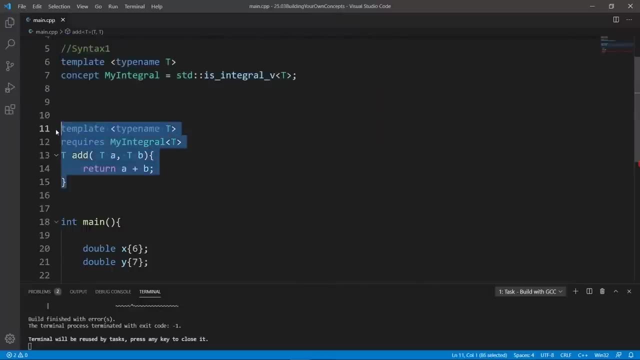 to evaluate this to false. hopefully you can see that you can really set up your own concepts using this syntax here and we can use our concept with all the syntaxes we have seen in the last lecture so, for example, we can take out the requires, close all together here and say my 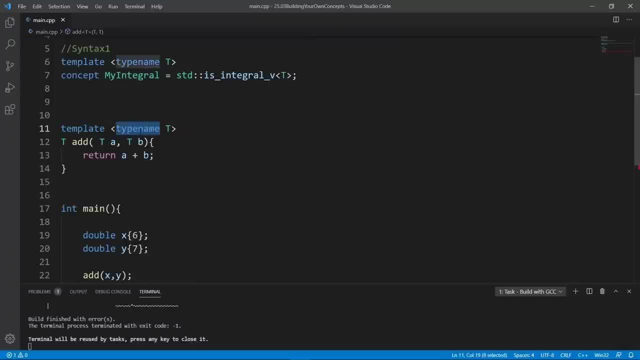 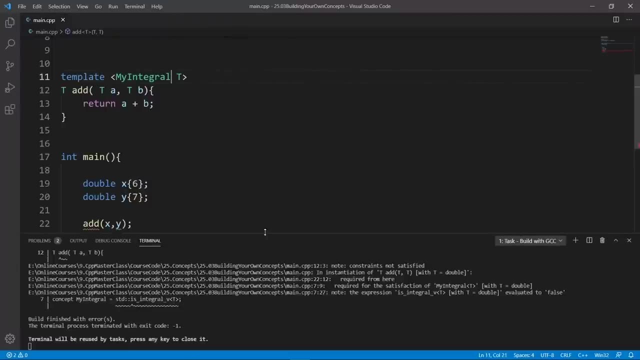 integral in the template decoration here. so we're going to say my integral and if we do this we're going to fail again because the concept is not going to be satisfied. we're going to have the same problem. we can change the syntax to use the auto syntax. but before we do that, let's change this back to. 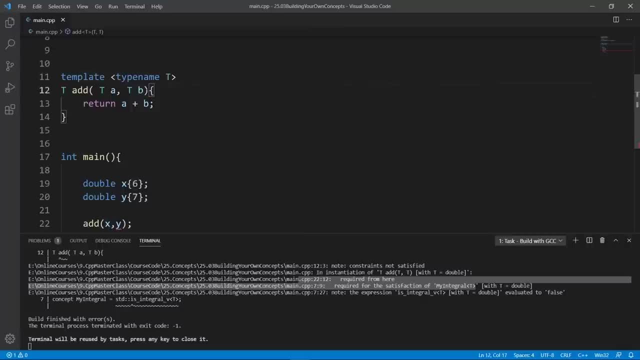 type name t and then put our requires close after the parameter list of our function template. we're going to say requires and we're going to say my integral and specify the template parameter and this is a valid function template with a concept applied to it. and if we both, again we're 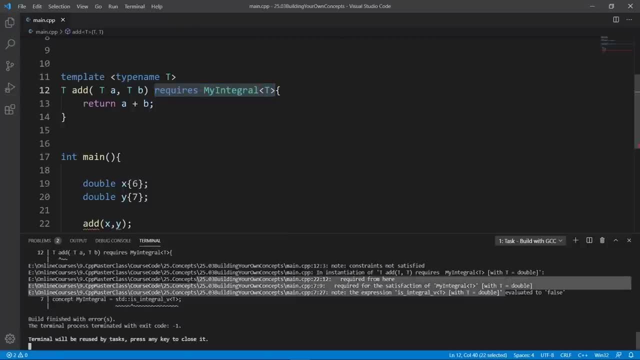 going to get the same compiler error. so you see the same compiler error and then we're going to the same and we can also use the auto syntax in ourotted library. winding conventional code. let's do that. we're going to take out the template declaration here. 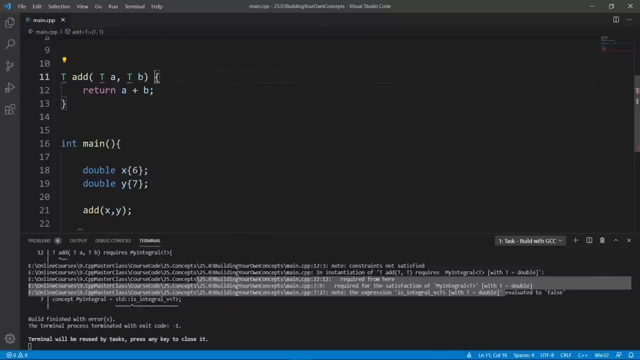 we're going to take out the requires close here and we're going to change our t to auto and that, the way we do that. we're going to say std, no, no std, we are using our own concept. so we're going to say my integral auto, this is going to work, and we're going to say my integral auto. and 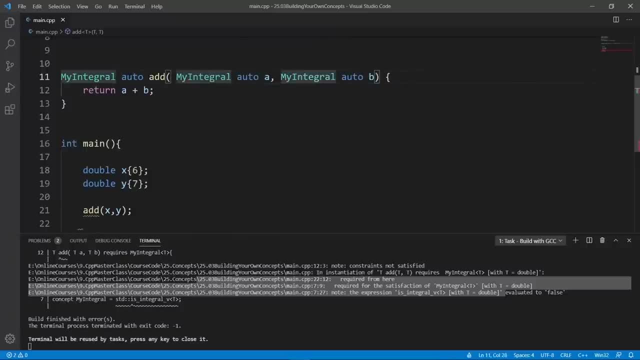 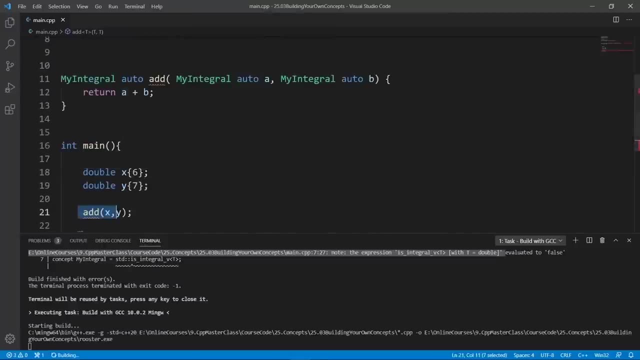 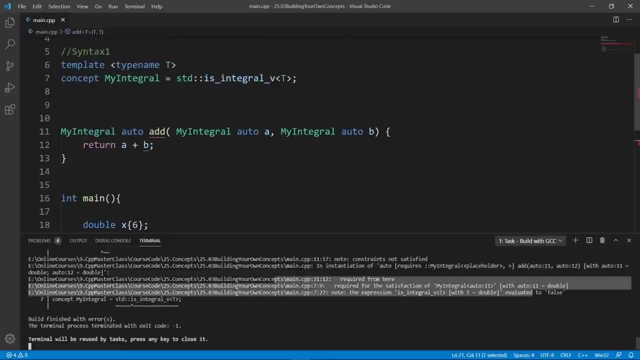 my integral auto here the moment we do this. you see that we have squiggly lines here because our concept is violated. but if we try and build again, we're going to use gcc to do that. the build is going to fail. you see that the same concept is violated and we are able to use our concept. 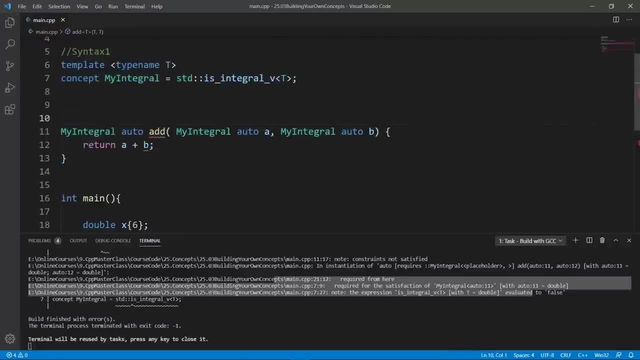 throughout the four syntaxes that we saw in the last lecture, and this is really cool. now that we have this, we're going to comment this out and we're going to see that we can set up concepts that have requirements spanning multiple statements or multiple lines. okay, let's go down. 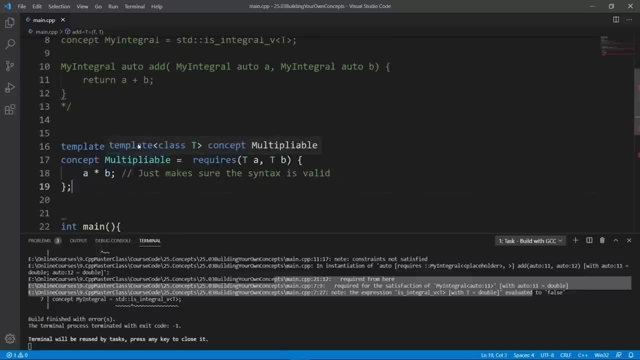 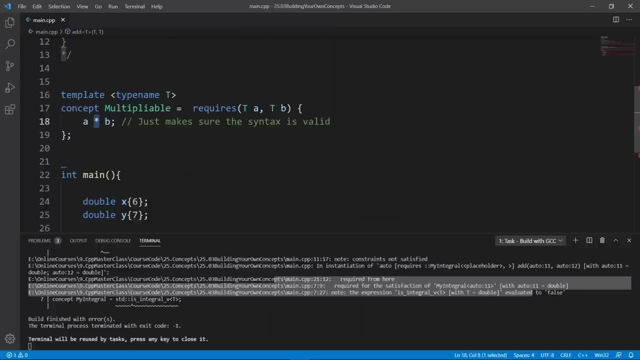 and do that suppose we want to set up a concept that is going to enforce for the template parameters to be multipliable with the multiplication operator we have here? we can use this syntax: here we're going to put in our template declaration, we're going to say concept, we're going 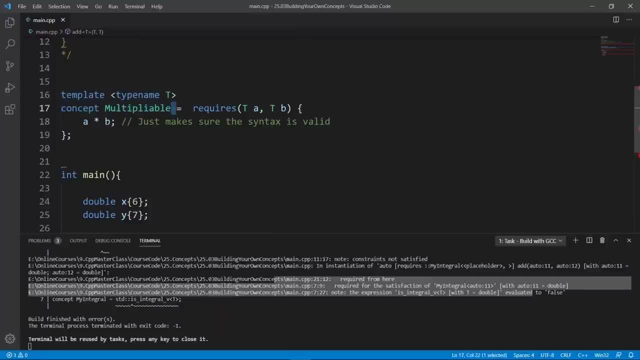 to say the concept name, we're going to put in an equal sign and then we're going to put in a requires, close with a our template parameters, and and after that we're going to put a pair of curly braces and inside the curlies we're going to put the requirements. for example, in this case we require for the template. 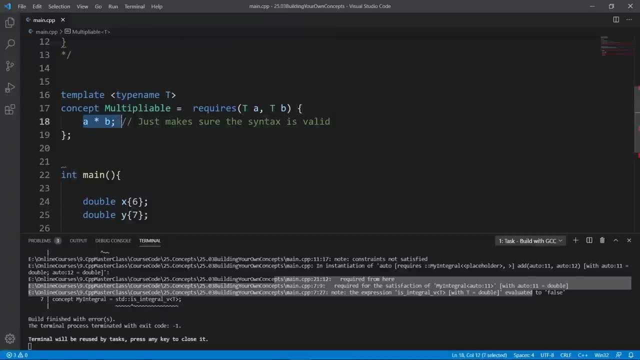 parameter here to support the multiplication operator between two of these types. if the multiplication operator is not supported, we're going to have a problem and this is the concept that is going to enforce that. one thing you should know is that this is just going to check that multiplying a and b is valid syntax. it's not going to check the value of a multiplied by b and 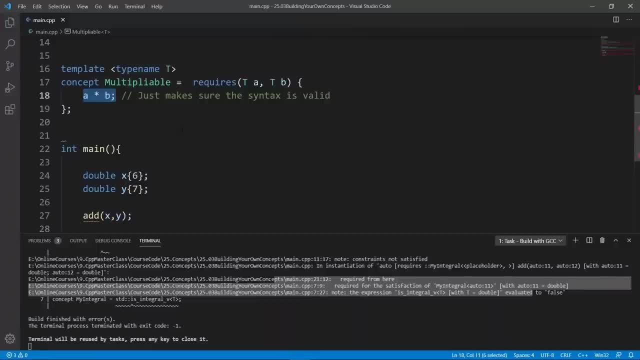 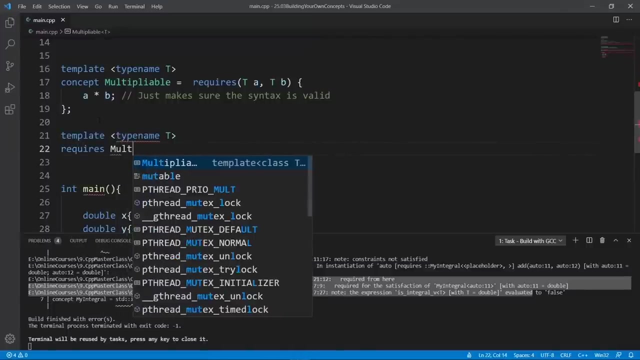 you should really understand this. now that we have this n, we can set up a function to use these two guys. why not use the function we have seen before to add two numbers? let's do that and we're going to put in our requires clause and we're going to require now to support the multipliable concept and 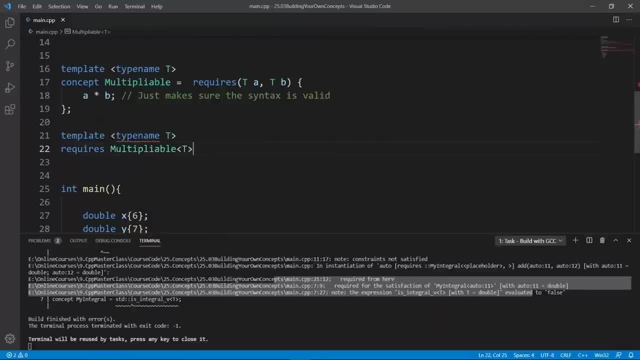 we're going to specify our template parameter. we have the concept n, so we can use that to do whatever we want. now we're going to say t add, and we're going to say t a and t b and we're going to return a plus b. this is the. 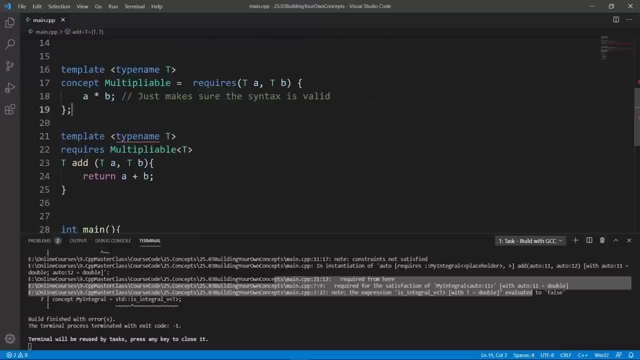 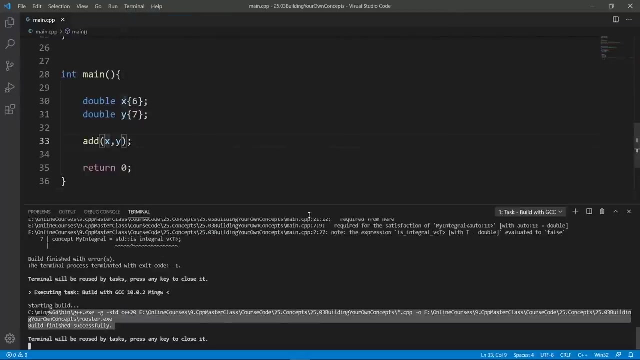 same function we've been using all along. okay, now we have our concept in place and we have a function template that is going to use this concept. let's see if we can add up x and y and see what we get. we're going to build with gcc. we're going to see that the world is going to be. 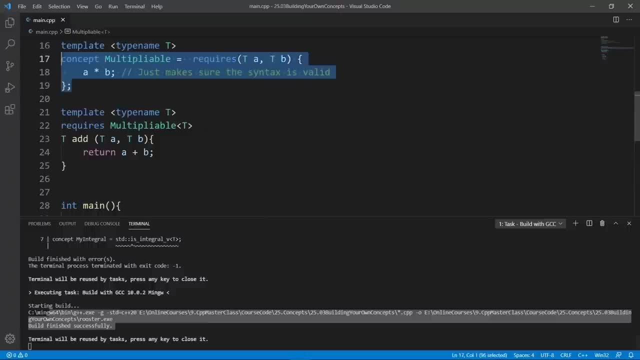 good because our concept here is satisfied. we are passing double types for our function template and it is legal to multiply two double variables. if we multiply two doubles we're going to get a value and that's going to be valid c plus plus syntax. but let's see what happens if we try to. 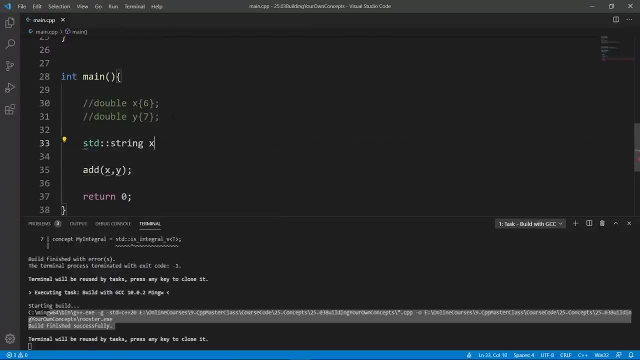 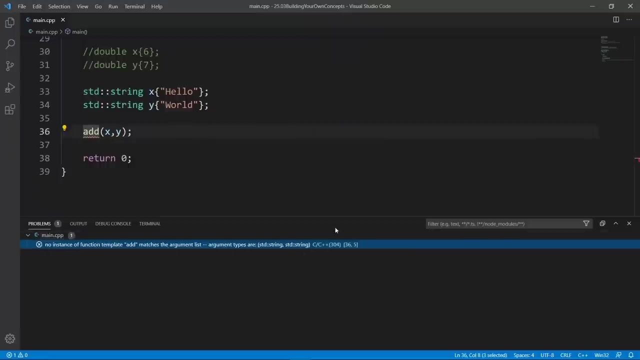 change our arguments to std strength. let's do that. so we're going to say x is hello and we're going to say y is world, why not? let's go down and put in our semicolon, and the moment we do that, you see that we have a problem and our visual studio code is not good at. 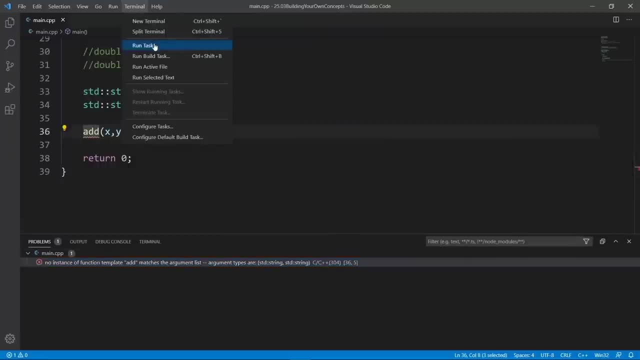 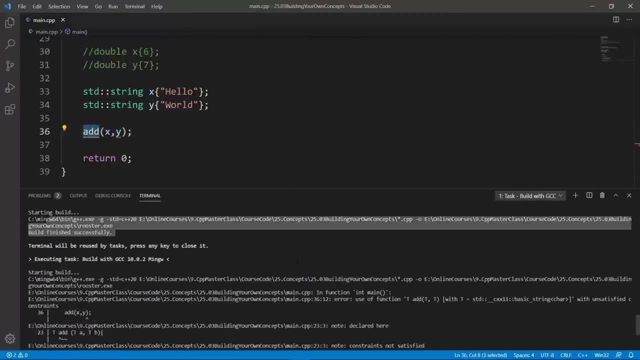 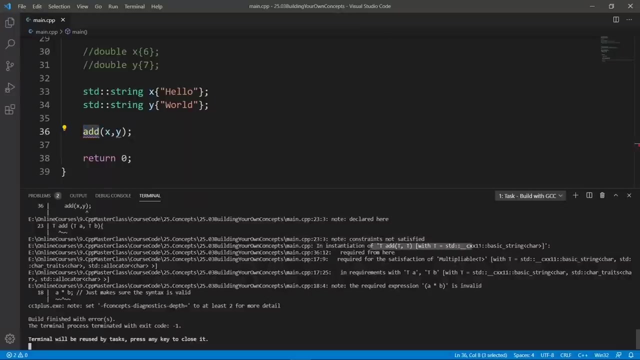 this yet, but if we go inside and run this through gcc, we're going to get that our concept is violated. let's look at the compiler error here. it's going to say constraints not satisfied and it's going to tell us that we are calling the add function with values that can't be multiplied. 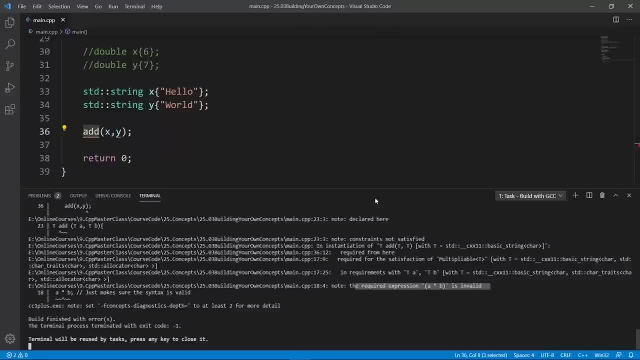 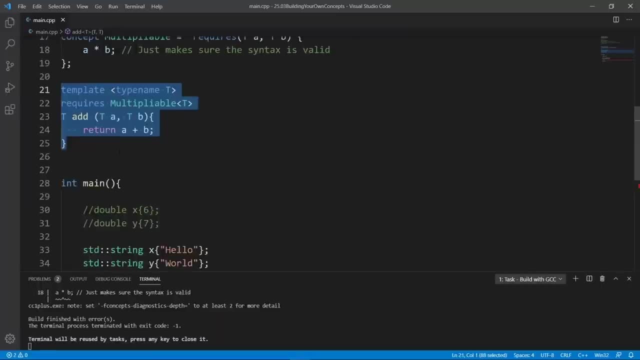 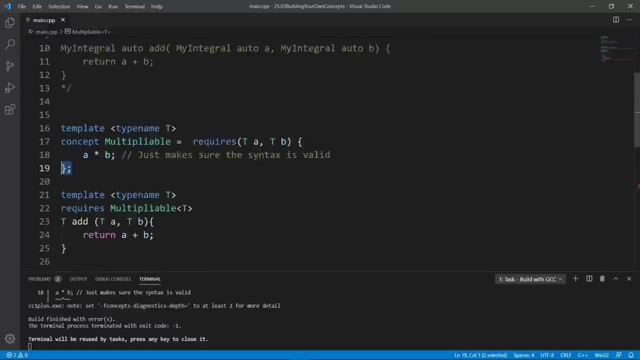 it's going to say: the required experience here is invalid, and this is how you can set up a concept like this and you can really use this to put constraints however you want on your function templates. but here we have just used one statement inside our concept. here we can even put in more, so to drive this home we're going to set up another. 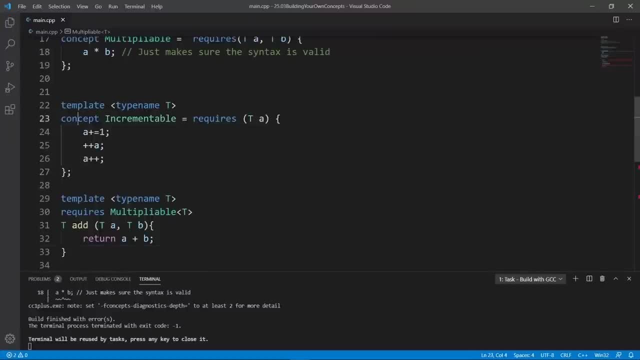 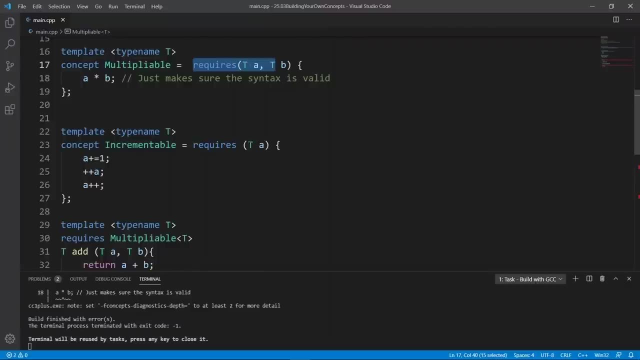 concept. let's go down and put that in place. the concept is going to be called incrementable. it's going to be using the same syntax we saw here, but we're going to be putting a requirement on the template parameter here to support incrementation and we want for every type. 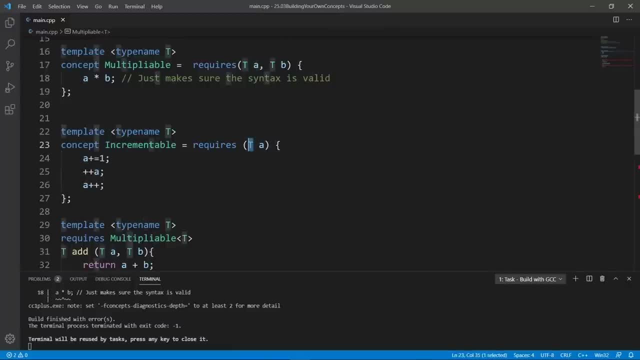 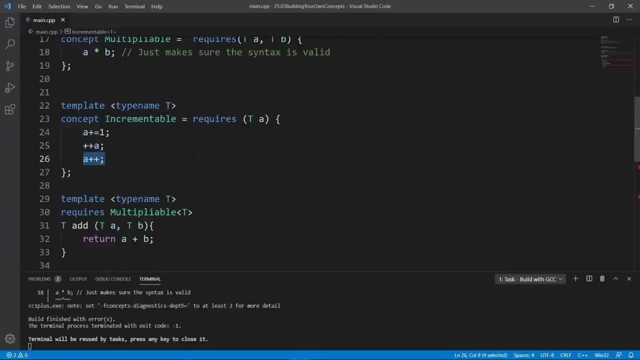 that goes in the place of t here. we must be able to say a plus equals one. this must be valid c++ syntax. we must be able to say plus plus a. this must be valid c++ syntax. and we must be able to say a plus plus. this must be valid c++ syntax. now that we have this, we can change our add function. 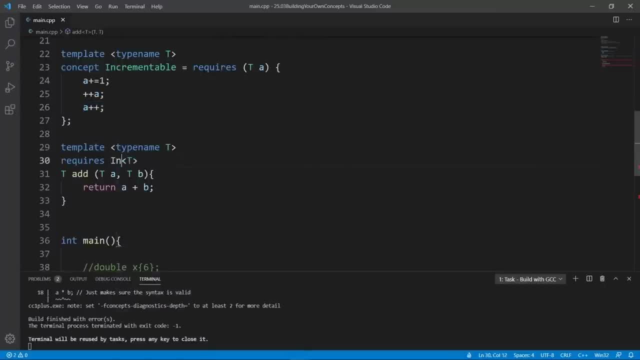 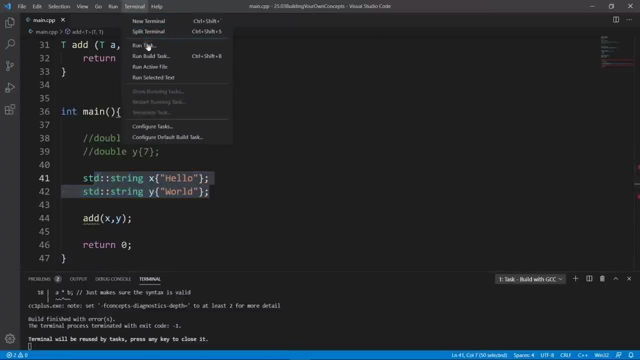 to use this concept. why not going to say incrementable? and now this function is going to be required to use things that we can increment on, and you see, it is failing already because we can't really increment strengths. what does that even mean? so let's build and show you the compiler error. okay, you see, incrementable is. 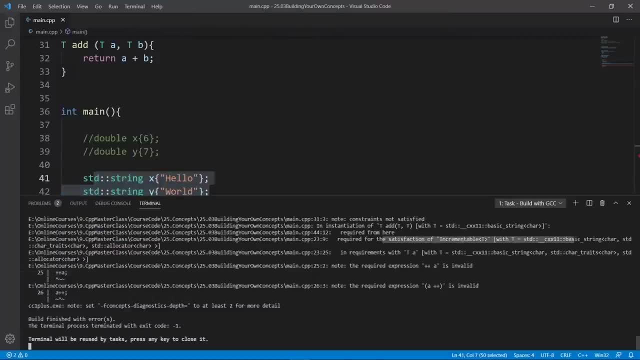 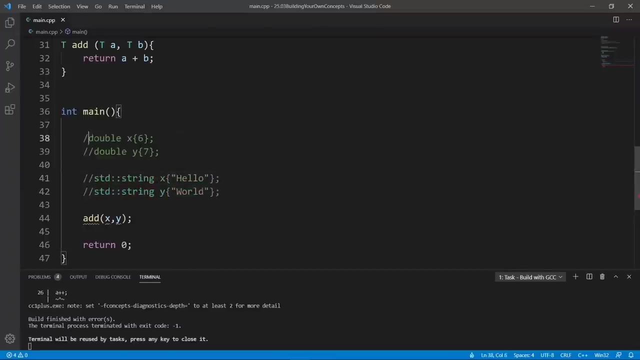 not satisfied and the required expressions aren't valid. you see, plus plus a is not valid, a plus plus is not valid and a plus equals one should not also be valid. but we're not seeing that here. but hopefully you see the message here that our concept is failing here if we comment out our strengths here and uncomment double. 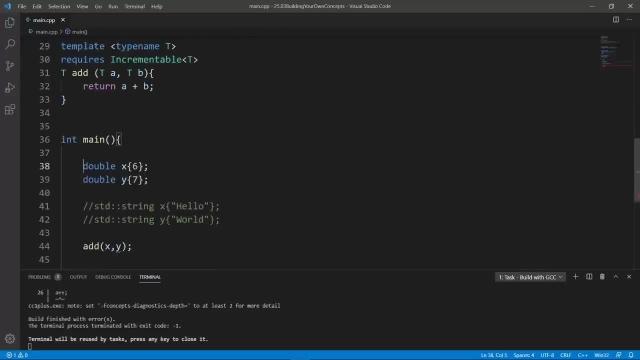 all these operations we have here are supported for the double type, so we should not fail here if we try to compile this, because the concept is going to be satisfied, let's use the gcc compiler to build. you see, the build is good. now we're going to use the gcc compiler to build the gcc compiler. 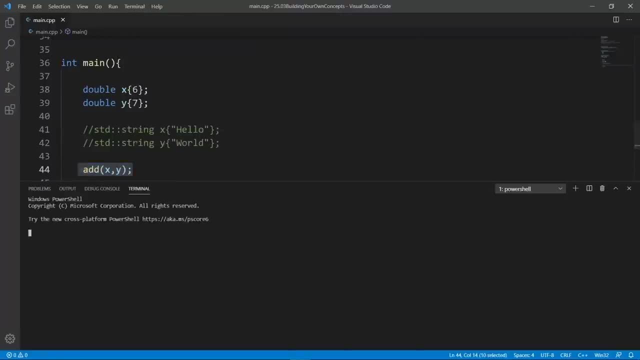 and we can clear and we can bring up a terminal to really see this, that our binary was generated. let's do the ir, we're going to see our rooster executable here and if we go down, let's say done. we're going to see that if we build again to bring this in consideration, clear run rooster. 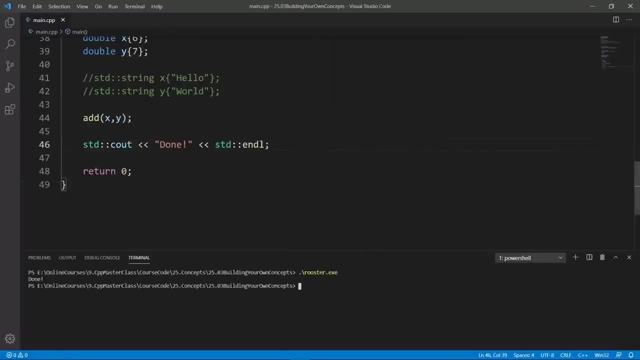 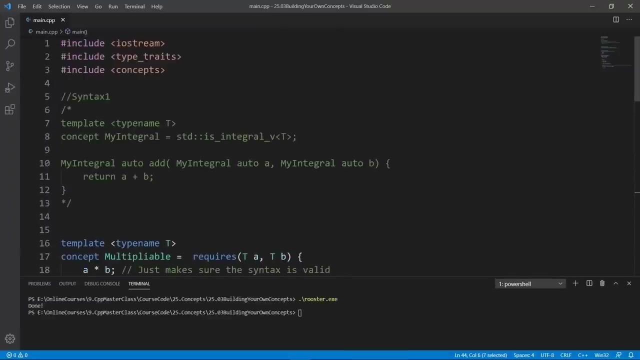 the program was generated and it is really running because the concept here is satisfied with our call using double arguments here. okay, so this is really all i set out to share with you guys in this lecture. i hope you know the syntaxes you can use to create your own concepts. you can either use 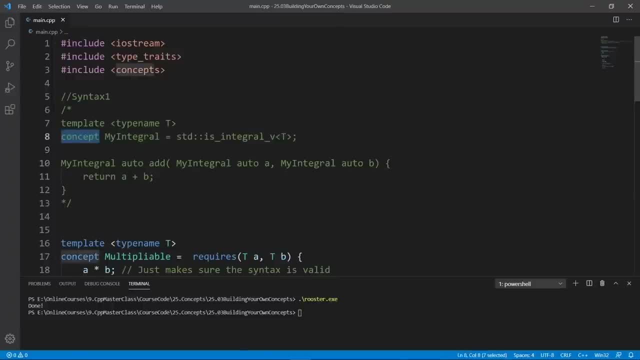 type traits, like we have seen here, and the syntax is to put the keyword concept, put in your concept name, put an echo sign and then specify your type trait here. this is going to work. if you need something a little more complicated, then you're going to use this syntax here. 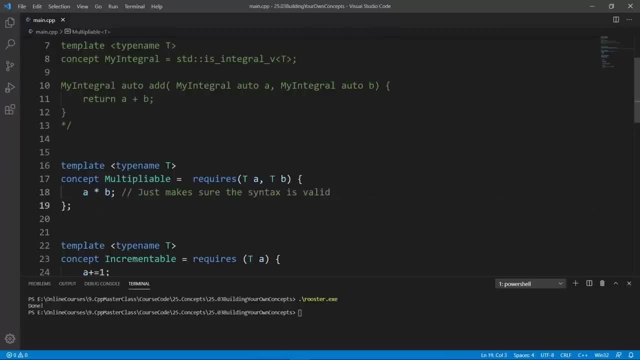 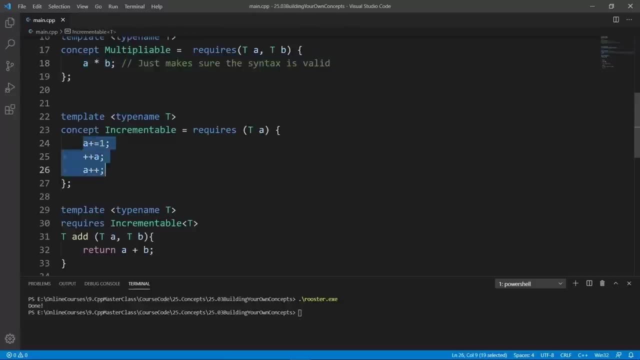 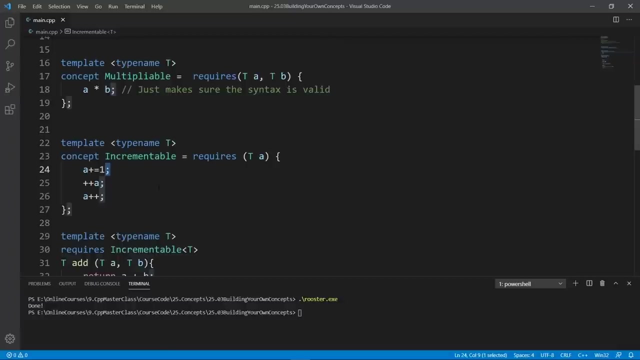 and put the query amounts for your concept in these curly braces. you can either put one statement, like we did here, or you can even put as many statements as you want. just remember to end them with semicolons. and another thing you shouldn't really take lightly is that this is just going to check. 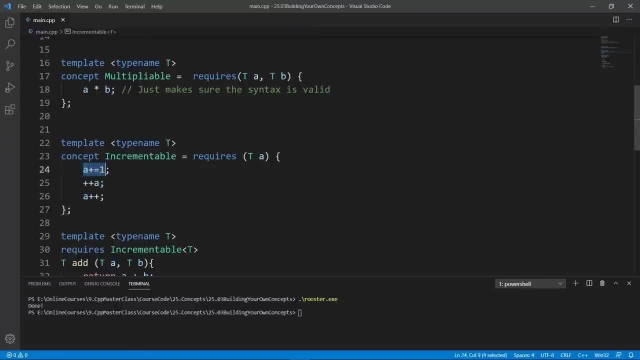 for syntax. it's not going to check for the value you get after you add one to a here, for example. it's not going to check for the value you get after you multiply b. it's just going to see that a multiply b is valid syntax for the types that our template parameter is using here. 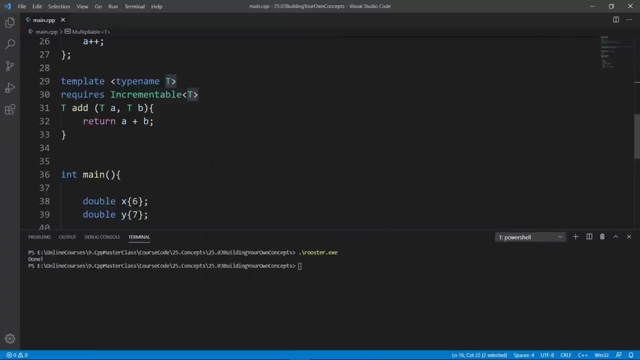 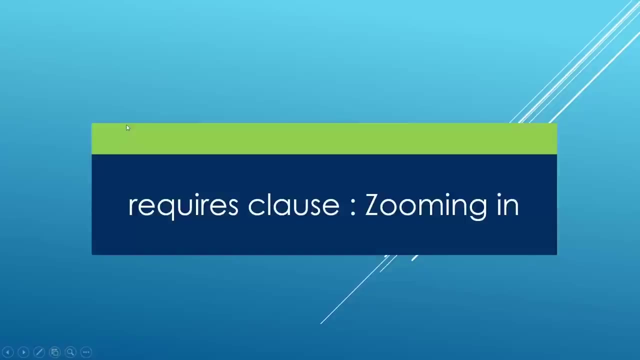 we are going to stop here in this lecture. the next one: we're going to zoom in a little more on the requires clause here. go ahead and finish up here and meet me there. in this lecture, we're going to learn about some more things we can do with our 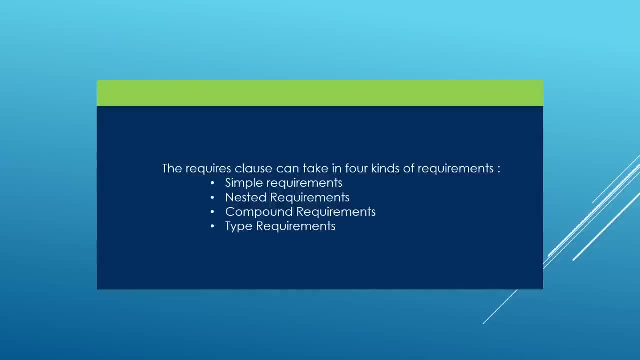 requires clause. but before we do that, let's look at the kinds of requirements we can put in our requires clause. the first one is a simple requirement, which is what we have seen so far. we can also do a nested requirement- and we're going to learn about this in a minute- and we can do a compound requirement. 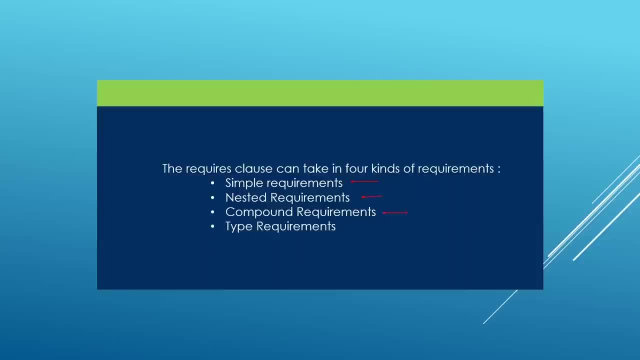 which is going to allow us to specify more things about what we require for our concept. there are also type requirements, but these are really advanced for the scope of this course, so we're going to talk about these in this course. what we're going to look at are these three. first, 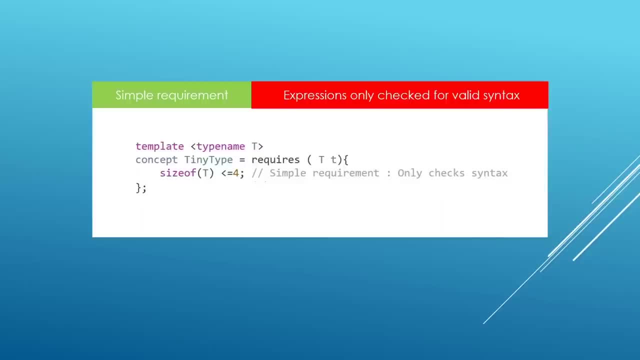 here. so let's look at a simple requirement. this is what we have seen already here. we have our template declaration. we have a concept declared. the concept name is tiny type. we're going to put in our requires clause, we're going to put in our parameter list and we're going to put in our curly braces. 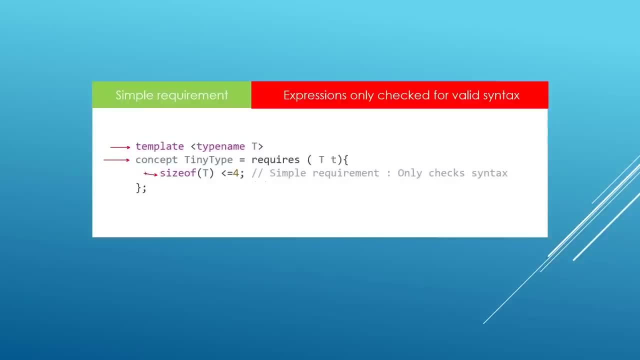 inside the requires clause. we have a statement here which is going to enforce that size of t is less than 4 and what this really means. it's going to check that size of t. the syntax here is correct and this can really throw people off. i have said this in the last. 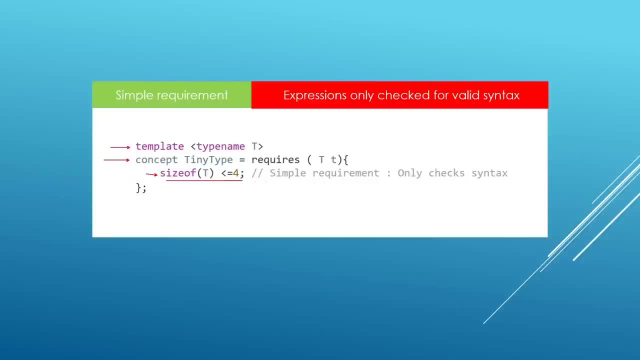 lecture. but i set up this little example to really drive this home and show you that if you are not careful, your concept are going to be really wrong. this is going to check for the syntax. so, for example, if we call a function template with this concept, with a car type, the concept is going to be satisfied, even if the size of the car 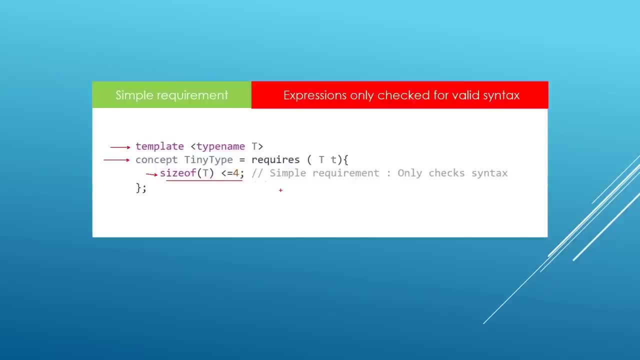 is less than 4, obviously, but that's not going to be the job of this concept here. this concept is not going to enforce for the expression here to evaluate to true, it's going to just check the syntax and if you pass something smaller than aET. 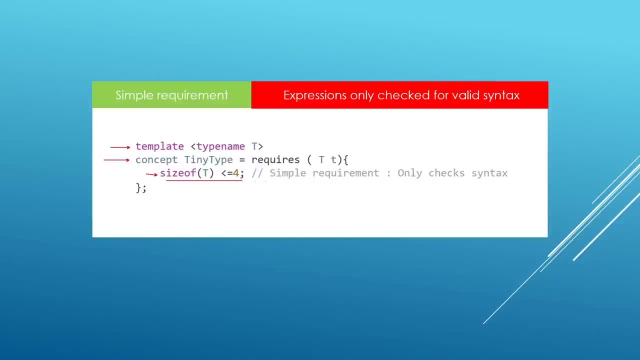 in a function template with this concept. this is going to be valid c plus plus syntax, so the ến concept is going to work. so now you must be asking: how can I enforce for the value of this expression to be true using concept? well, for that you will. 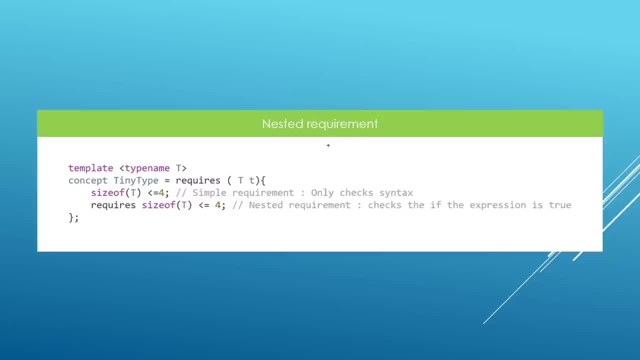 have to use nested requirements and a nested requirement is going to have another requires keyword inserted in front of it. now, if you use the syntax like this, now this is going to check that size of T is actually less than 4. if it's not less than 4, this is going to return false here and the concept is: 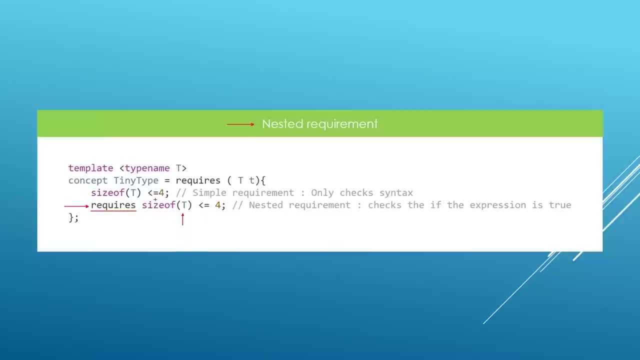 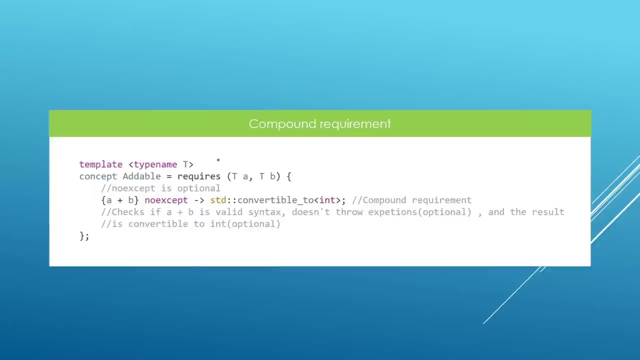 going to fail, and this is how you can use nested requirements to enforce for some expressions to be true in your requires clause. another kind of requirement you can set up for your concept is the compound requirement, and this is going to allow you to check if something doesn't throw an exception. you. 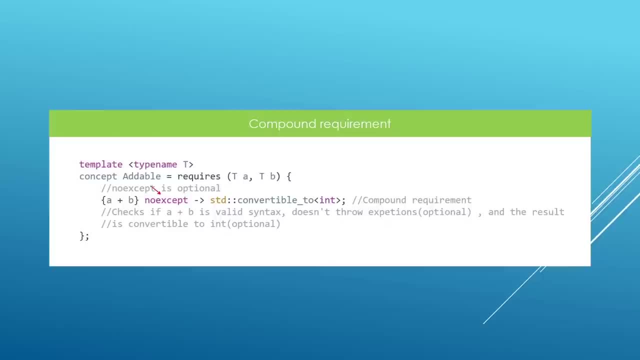 can do that using the now except keyword, but we're not going to use this now because this is not. you can do that using the now except keyword, but we're not going to use this now because this is not in scope for what we can do at this point in the course. but you can also. 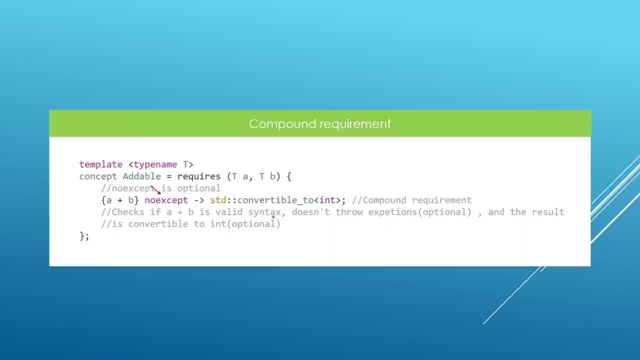 check the return type of an expression and enforce that it satisfies some type trait, for example. so here we are saying for our concept: and if we pass in two parameters, the syntax for adding a and B must be correct and supported for those types. but the result of a and B must also be convertible to ant and you can. 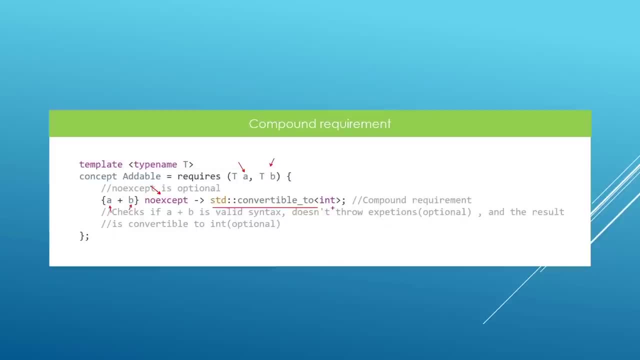 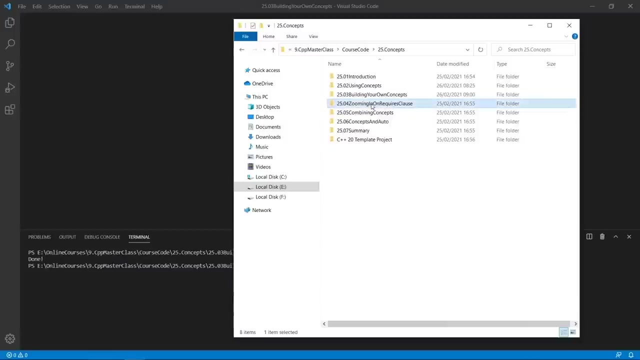 do something like this, and this is going to work. you can enforce these kinds of plants using compound requirements. okay, now that you know about these kinds of requirements, you can put in your requires clause. let's head over to Visual Studio code and play with us a little more. okay, here we are, in our working folder, the current. 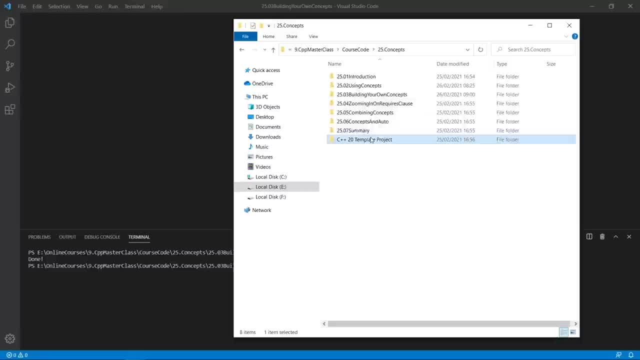 project is zooming in on requires clause. we're going to grab our template files and we're going to put them in place and we're going to open that in Visual Studio code pretty quick by dragging and dropping here. this is going to open up our folder. we're going 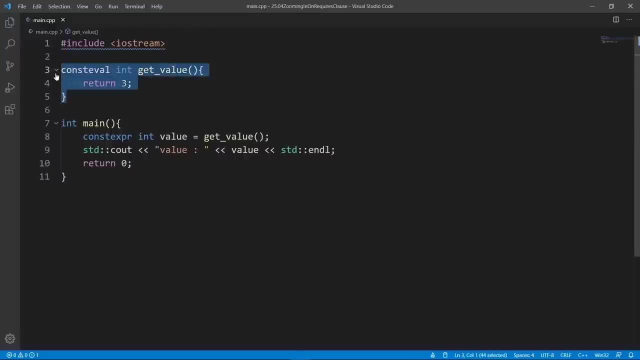 to do the usual. we're going to close the pane here, we're going to clean things up a little bit and we're going to include our concepts library. let's do that. we are going to set up a simple concept for going to say template and we're going to 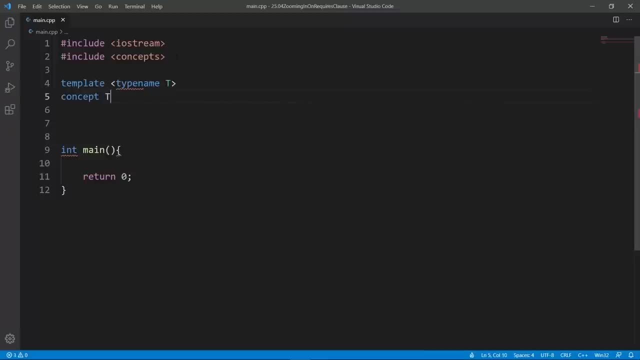 say what the concept is. the concept is going to be called tiny type and we're going to say what makes this concept a tiny type. we're going to put in our requires close and we're going to put in the template parameter- call it t, why not? and we're. 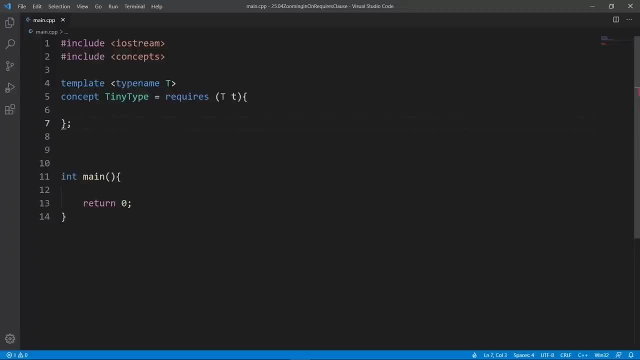 going to put in our closing semicolon here now. what is going to make this concept a tiny time is that the size of the template parameter view is going to be less than four. let's suppose we are doing the function and we want it to use for integral types that are smaller than four bytes. 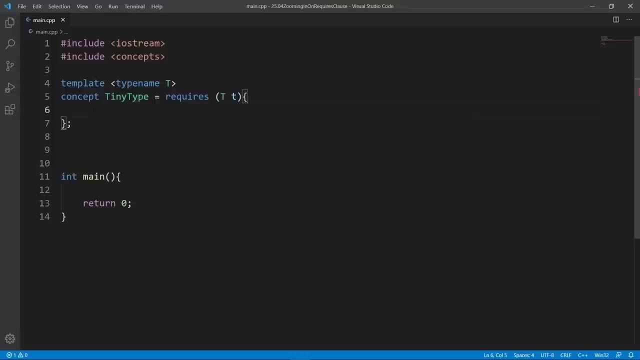 in memory. suppose you want to do this and it is useful in the problem that you are trying to solve. in c plus plus the way we can enforce this. we can say size of t is supposed to be less than four. let's say size of properly can't type, can i okay? the moment we do this, you're going to see that. 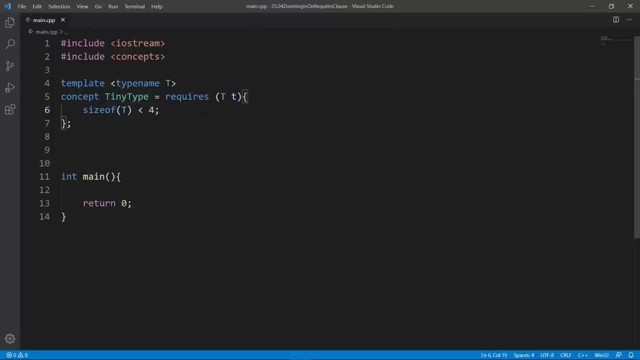 this is valid c plus plus syntax, so we're not going to have any squiggly lines. but what you should know is that this is a simple requirement in c plus plus concept, and what this is going to do, it's just going to enforce the syntax of what we do here. what we put here must be valid c plus plus. 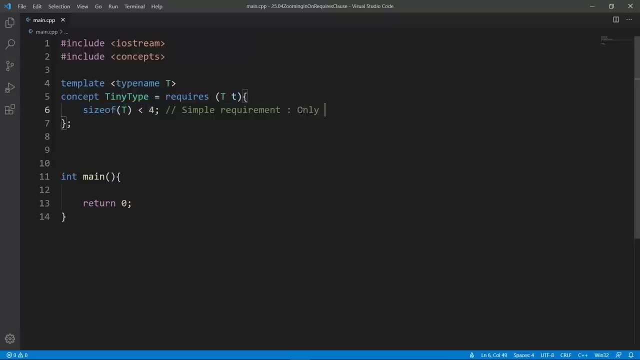 syntax, so only enforces syntax. this is what you should really remember. okay, now that we have this end, let's try it out and show you some problems you can really run into. we're going to set up two character variables. we're going to call the first one x. we're going to initialize this with: 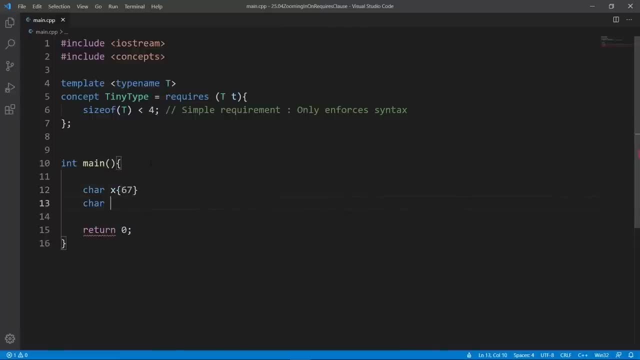 57, why not 67? and we're going to put in the other variable, which is going to be to be y, and it's going to have a 56, and you can put in whatever you want. just make sure that you are within the range of the car type, which is between 0 and 255, if you remember. okay, now that. 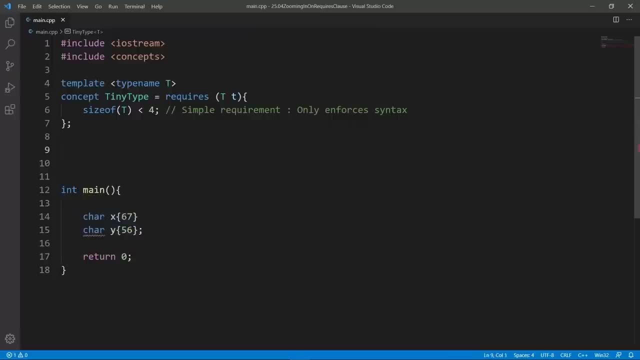 we have this n. i realized we don't have a function. we can try this on. let's set up another function pretty quick. we're going to say tiny type auto. we can do that, you already know the syntax. and we're going to say: add tiny type auto a and a tiny type auto p. and we're going to set up another function pretty quick. we're going to say: tiny type auto. we can do that, you already know this syntax. and we're going to say: add tiny type auto a and a tiny type, although is it a little less than the canine type,2585iendo 12 róż been RM. ignorishing this syntax. it's going to say 7m, 80%N reaching 5m, 65- outro 8m. 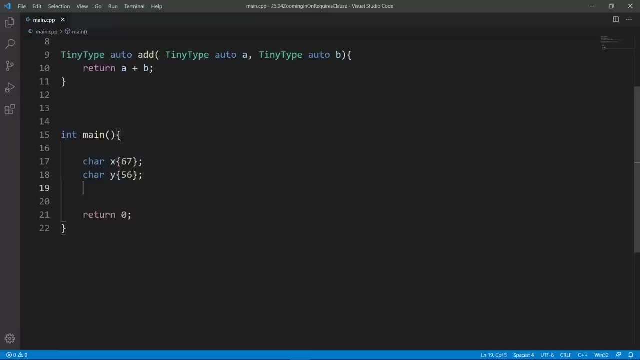 we can do that and we're going to return a plus b. now that we have this, let's say a and b down here and call this function. we're going to say x and y and we're going to try and compile this program. and it is going to compile fine, because the type we are using to call the function, which is car, 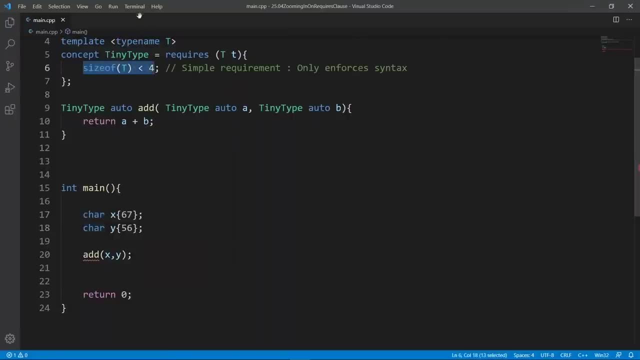 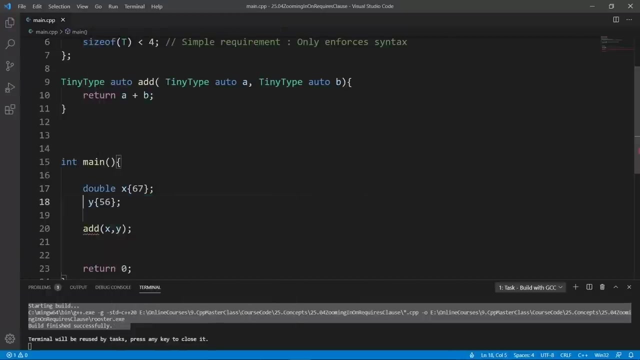 its size is going to be less than four. okay, so this is going to work and it is going to compile. let's build with gcc. you're going to see that the build is good. let's try and change the type here to ant or even double. you know, double is eight bytes in memory, so we expect this to probably give. 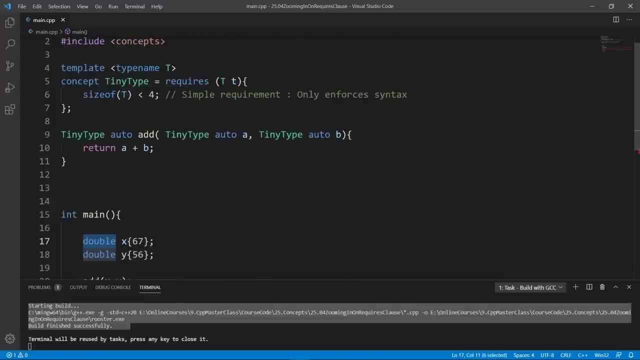 us something wrong. double type is eight bytes in memory. so we expect the size of t here to be false, because the size of t is going to be eight and eight is not less than four. this is going to be false. so some might expect this concept here to fail. but let's try and really prove you wrong. 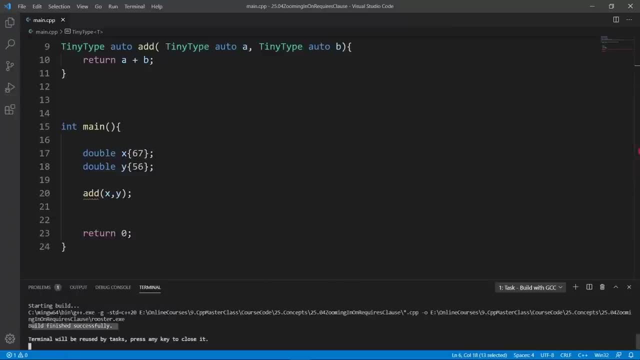 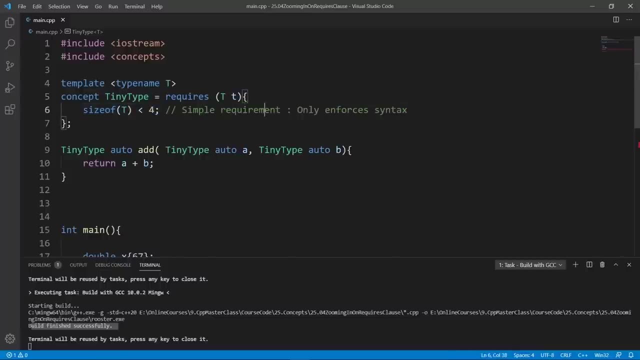 we're going to build with gcc and ucc. it's building successfully. what this is really doing is that with simple requirements like we have here, c++ is only going to enforce. for this to be valid c++ syntax, and size of t is less than four is going to be valid c++ syntax, even if this expression here evaluates to false. 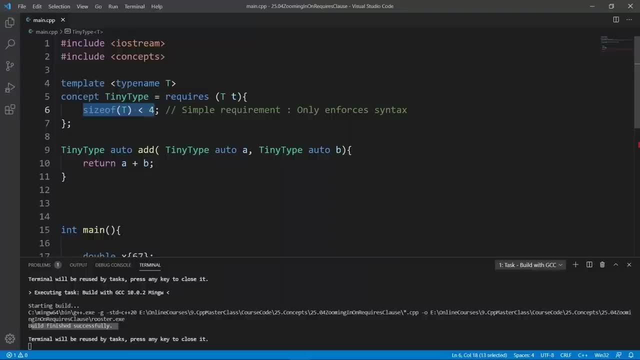 this is not going to enforce for the value of this expression to be false. you can't do that with simple requirements. what you will do is check that this is valid syntax. now what do we do if we really want to enforce that size of t should be? 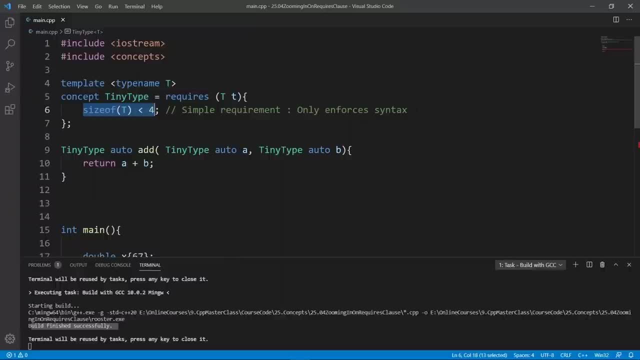 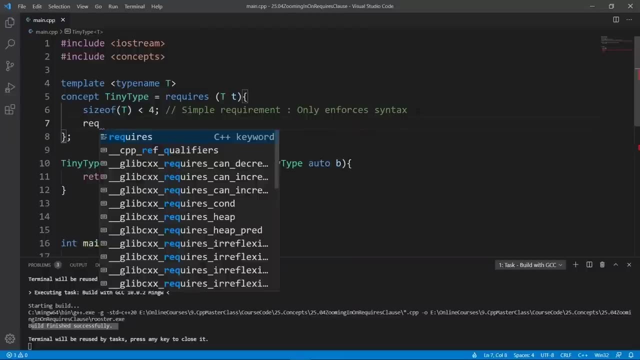 less than four. if you want that, you should use nested requirements, and the syntax to do that is really simple. we can go down here and put that in. we're going to say requires. we're going to add a requires keyword in front of this. then we're going to put our expression here. let's copy it. 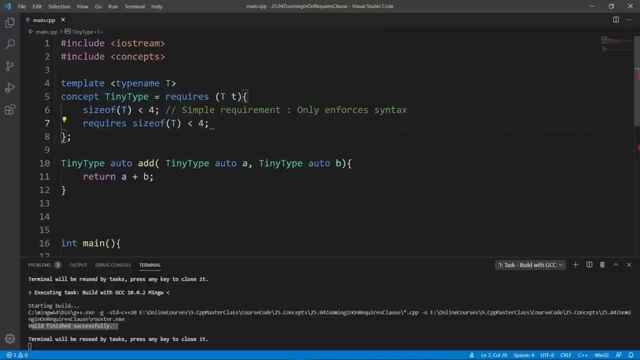 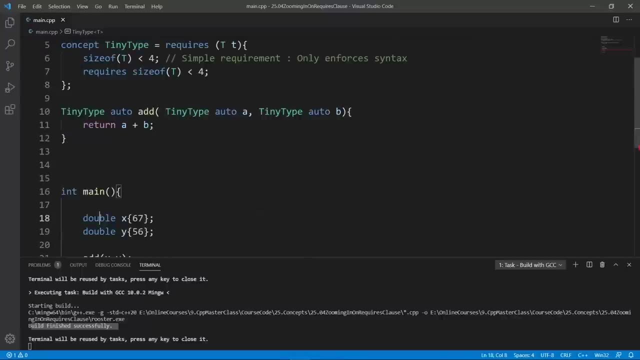 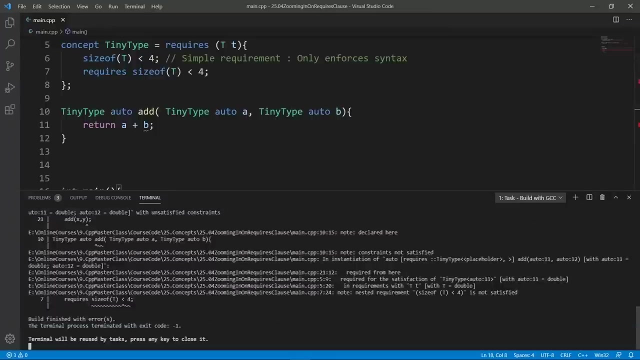 and put it in. i don't want to type this again. the moment we do this now, compilation is going to fail. if we pass a type whose size is not less than four and let's try and build again, you're going to see that the world is going to fail now and we're going to have a failed concept, and you see, 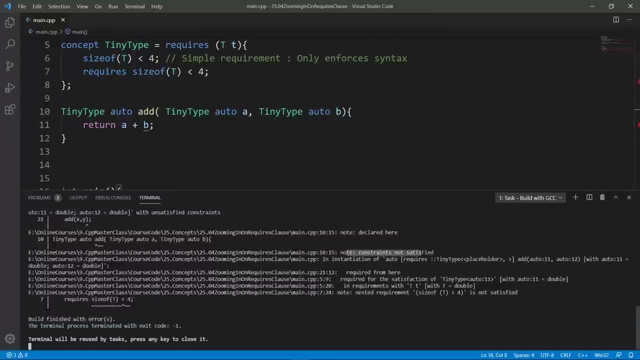 world finished with errors. we have constraints not satisfied and if we go down here we're going to see required for the satisfaction of tiny type auto. and we passed in a double type whose size is eight bytes in memory and it is less than four bytes you see. 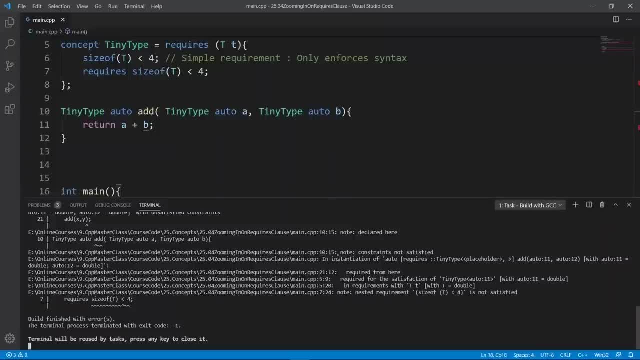 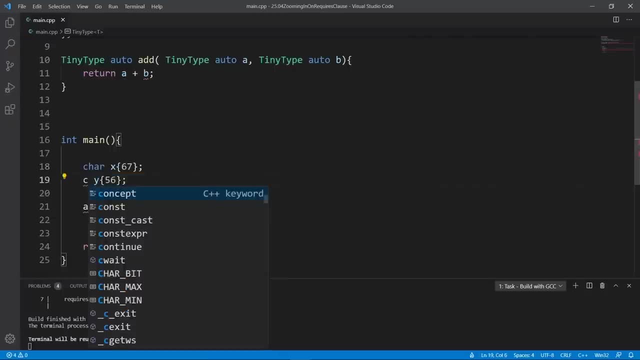 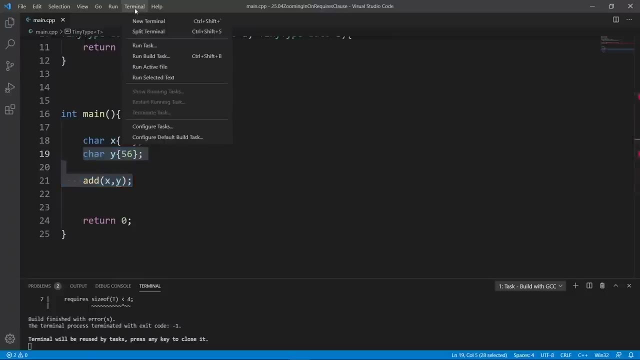 the requirement here, it is not satisfied. we can do this using nested requirements. okay, if we go down, for example, and change this to car- some people call this char, but i call this car. that's my habit- if we change this to car and try to build again, you're going to see that it is going to world. 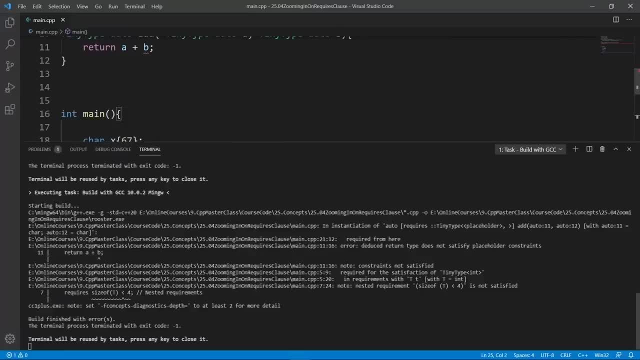 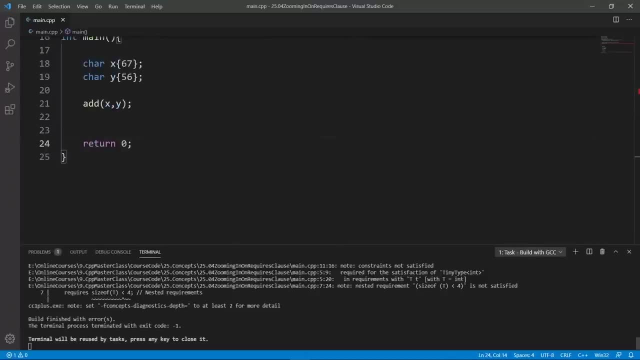 fine, because now what is wrong here? let's see what we get wrong. we are getting a compiler error here. what is the problem? it's going to say: let's go up and try to analyze this a little bit. it's saying: deduce the return type does not. 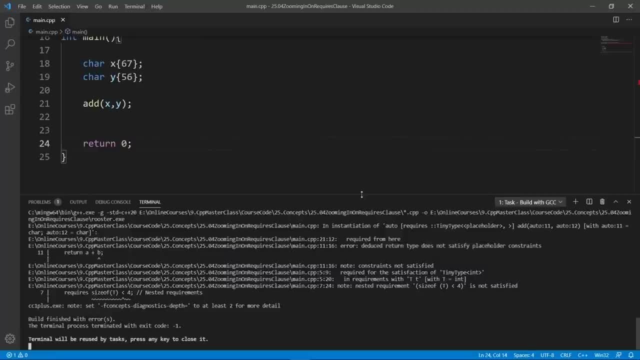 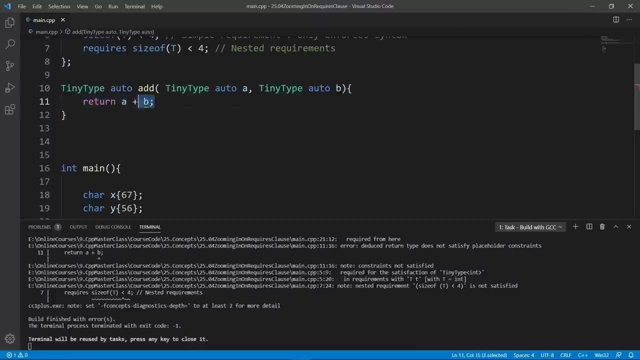 satisfy placeholder constraints and we are requiring for the return type of this guy to be tiny type. uh-huh, i think i know what the problem is. the problem is the arithmetic operations, like the addition we're doing here, are not supported for types which are smaller than ant. ant is the. 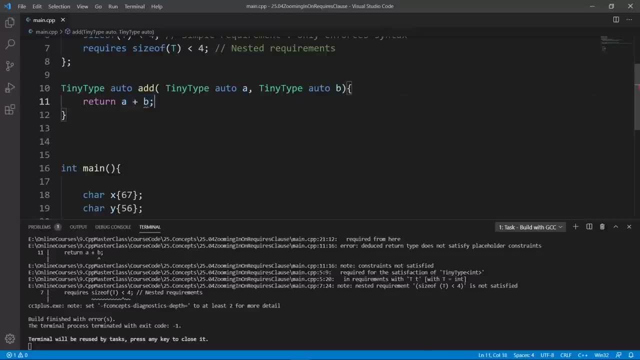 smallest type we can use with arithmetic operations. so what the compiler is going to do is going to do implicit conversions from car to ant and inside here what we will have are going to be ant. the result of this is going to be ant and the return type is going to be deduced to be ant. but ant is going to violate the requirement we have here. 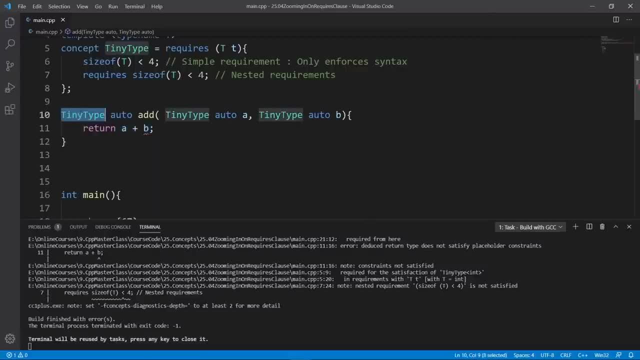 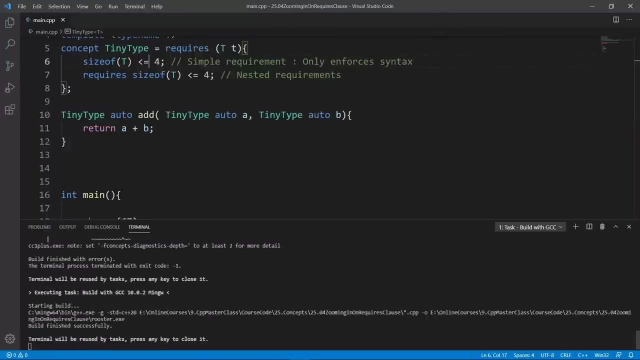 which is saying that the size of tiny type here should be less than four and the return of ant is not less than four. so we can try and fix this by putting an equal sign here and i think it's going to work. let's do that and build again. this is a good learning experience. 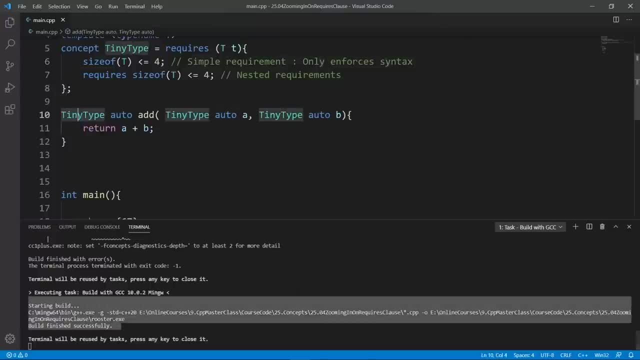 and now you see that the build is going to work because now the return type is going to satisfy our requirement. so let's prove that we are getting a net out of this. actually, we're going to do auto result and we're going to say equal and grab the result of this guy. we should. 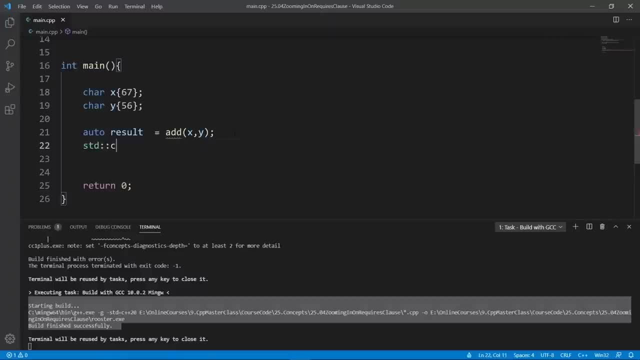 really prove these things, and after this, we're going to print the results. we can do that, and we can even go further and print the Ahawang result from our equivalent filter. we can do that, and we can even go further and print the title of this kid. we should really prove these things, ialfagh. actually we could put something in this. we could do this hotel package. so this is the point in the overal IFAW her. so there we need you just please send this item to us. that level my Joshua Obama, before this. then I'll text you the answer to this question. to aff compound here. 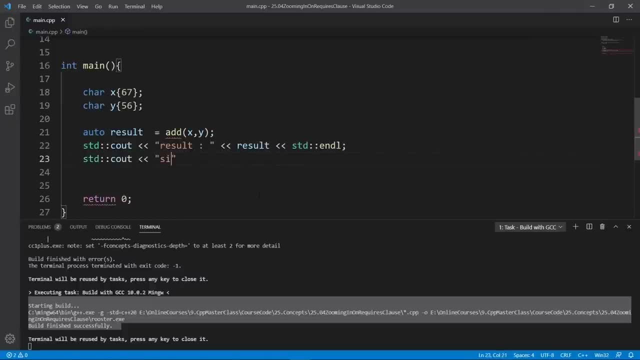 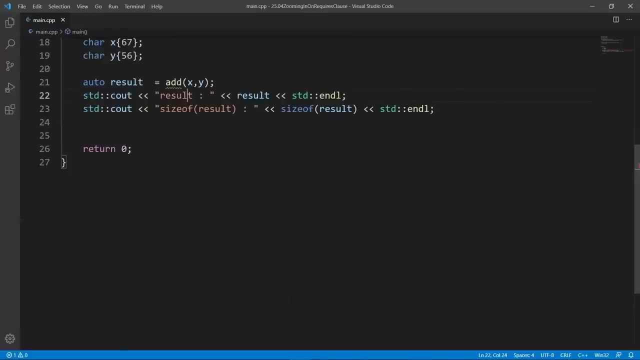 print the size of result here. so we're going to say size of result. okay, now that we have this end, we can build with gcc and the world is good. don't mind this quickly line. it is probably visual studio code messing with us. you see that the world is good. we can now bring up a terminal. 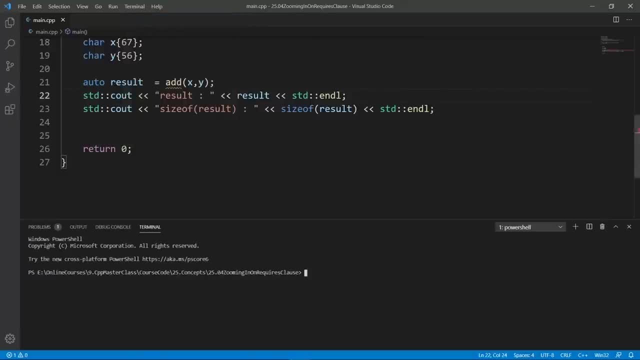 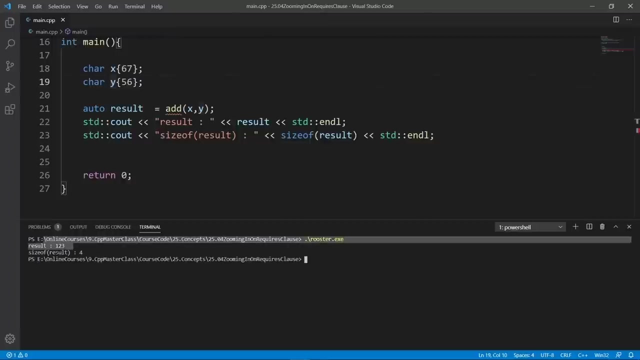 and run this and see the size of the return type and really prove that the compiler turned that into a net, even if we called our function with car arguments. this is interesting, so clear and run. rooster- now we're going to see results- is going to be 123 and the size of the result is 4. 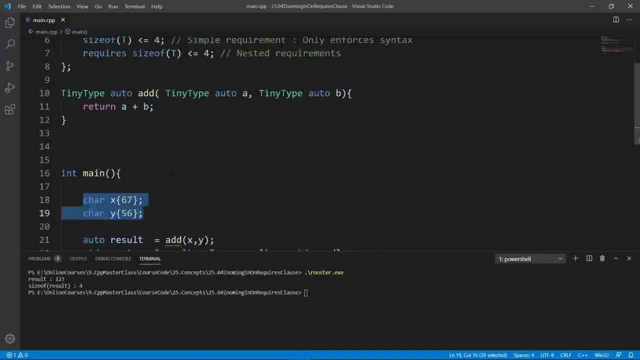 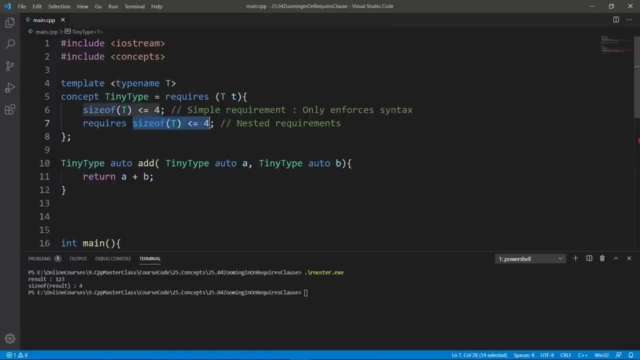 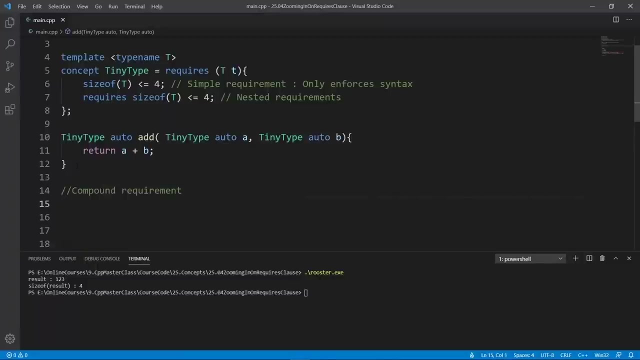 even if we passed in car types as our arguments. okay, so hopefully this proves that you can set up nested requirements to enforce- for the expression here to be checked. another type of requirement you can do is a compound requirement. let's put this in and we're going to put in a simple example. to drive this home, i think i should take this. 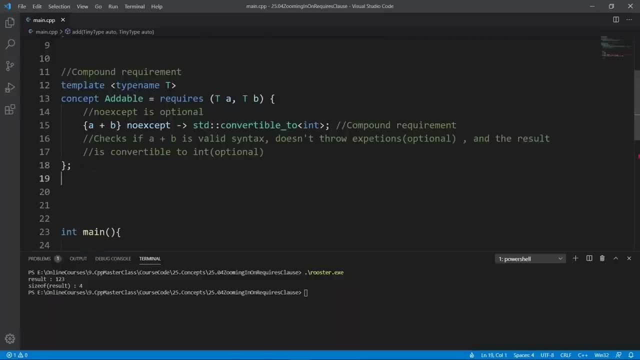 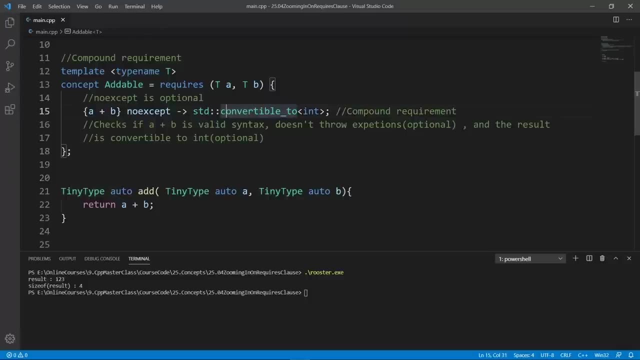 function and put that below our concepts. so a compound requirement looks like this: you put your expression in acrylics like this, and then you can even put requirements on the values of the expression. for example, we can enforce that the value of a plus b here should be convertible. 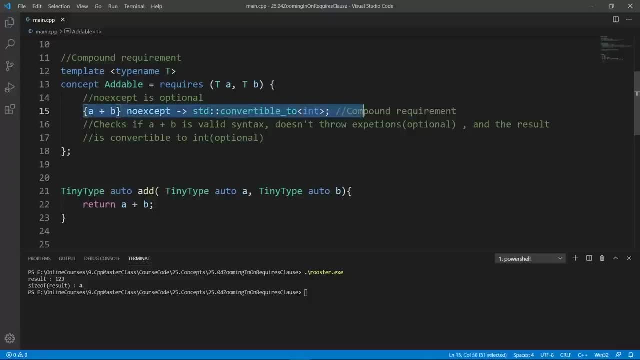 to ant if it's not convertible. to end, the concept here is going to fail. this a compound requirement. you can even put no except keywords in here. but we're not going to go this far because we haven't really learned about exceptions. so for now i'm going to take this: 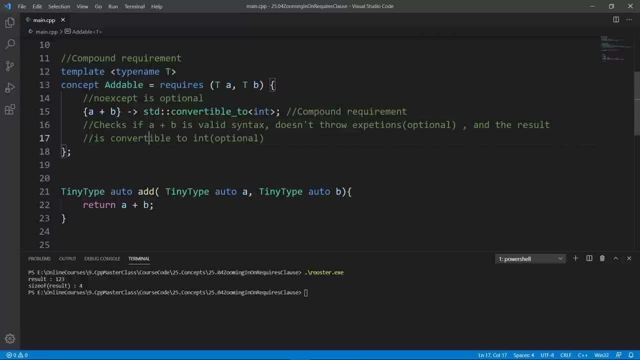 out. i just wanted you to be aware that you can do that, now that we have this concept- and let's play with it and see how we can make it break things- we're going to change our concept to addable. let's say edible here, and we're going to say edible and we're going to put in our car types. 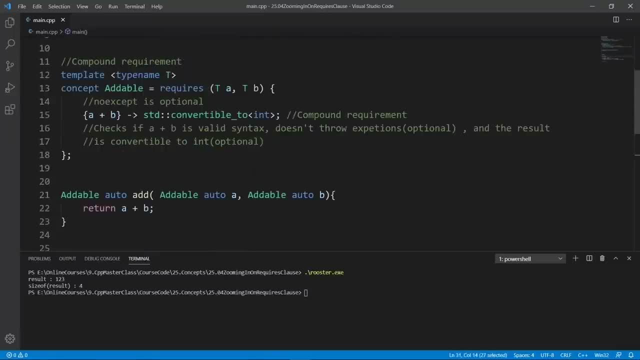 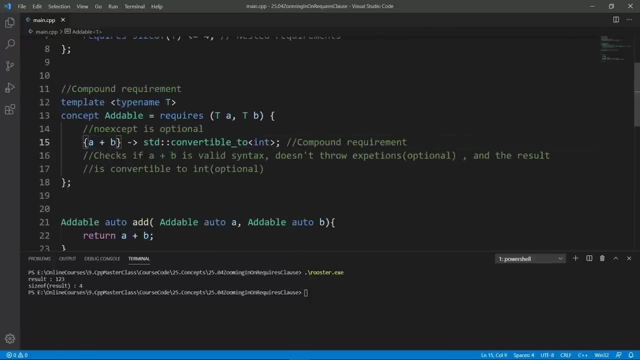 here and it is going to stay work because we can add two car variables and this is going to work because we can add two car variables and this is valid syntax. what we're going to get out of that is going to be an entity because, remember, the compiler is going to insert in: 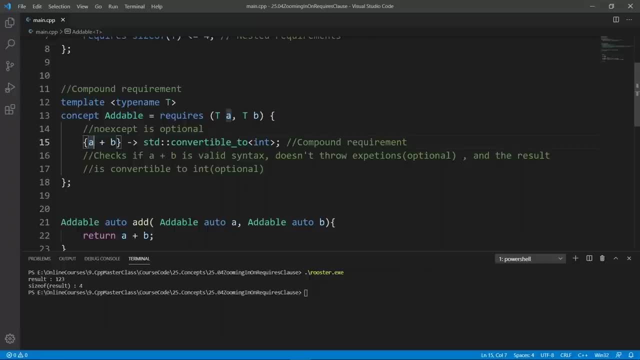 places conversions from core to end, because it can't really add two car types. ant is the smallest thing you can do arithmetic operations on, so the result of this is going to be an end, so a. the result of this is going to be an end, so a. 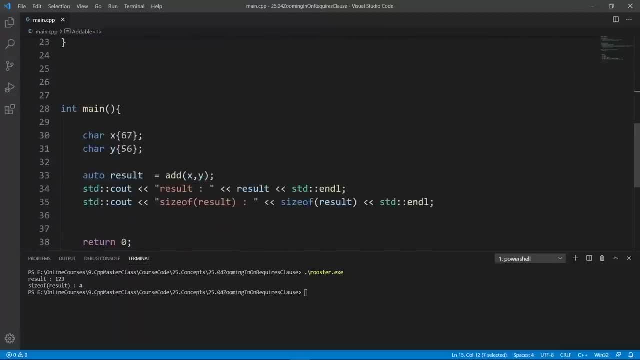 int is convertible to an int. this is going to work. let's build and show you that this is going to work. we're going to build this with the gcc. you see it build is good. we can try and run this and see what we get. after calling the function, we get result is 123 and this is going to be the size of. 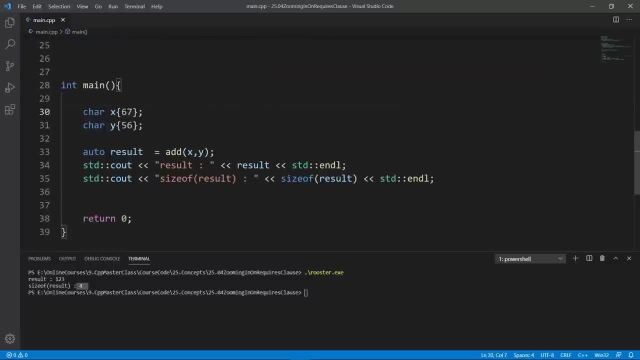 four, because we get an int out of this. let's try and change this to double and see what we get. so double, let's say double here, and if we build, we expect this to work, because adding up two doubles is going to give you a double and we're going to return a double from this function. 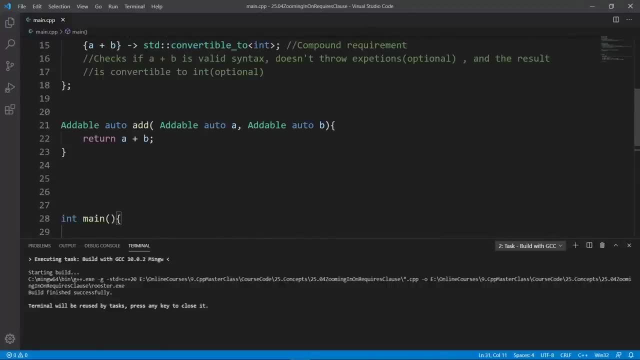 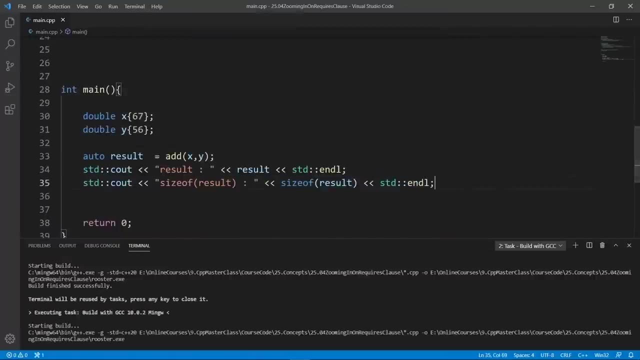 and a double is convertible to a net. so we're going to return a double from this guy and this should say 8. now, because that's what we are returning from the function here. let's build with gcc. you see, the world is good, we can clear and run rooster. this is going to say size of result is 8. 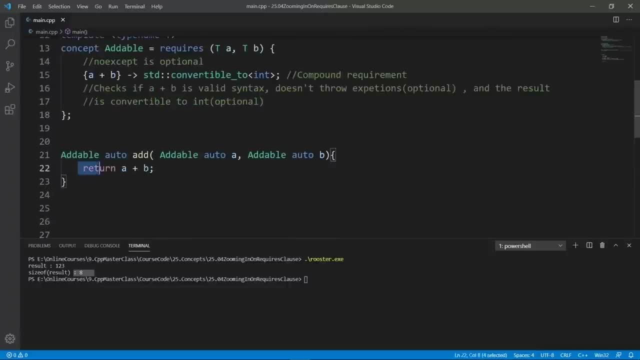 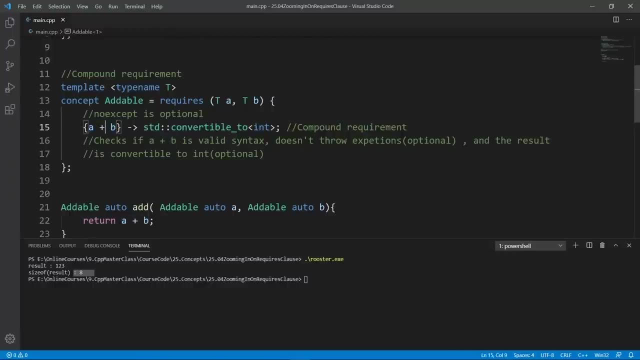 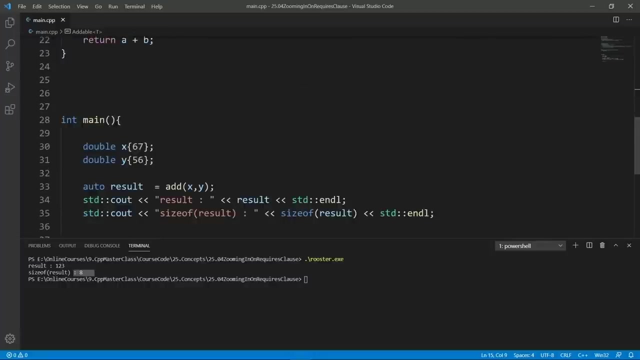 because now what we are returning is going to be a double from this function here, and double satisfies our concept. adding up two doubles is valid syntax and what we get out of that is going to be a double, and the double is convertible to a net. this is going to work. let's try and change our 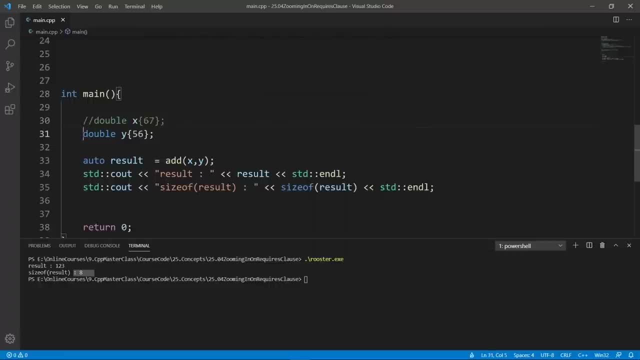 parameters here to strength, we're going to comment out our x and y variables here and we're going to set up two strings. we're going to say std strength x and we're going to say hello. and you know what we're going to say in y. we're going to say std strength y and we're going to say world, why not? 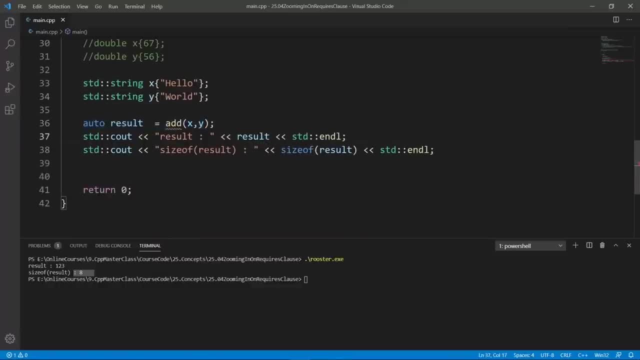 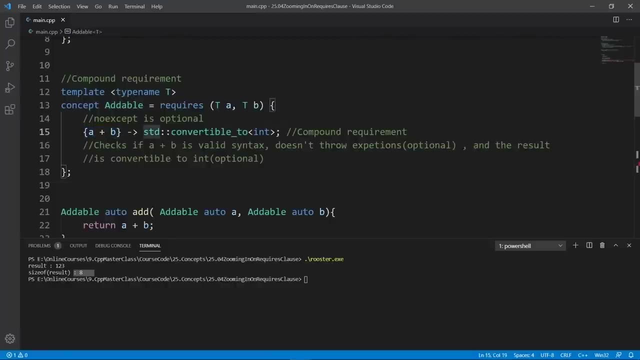 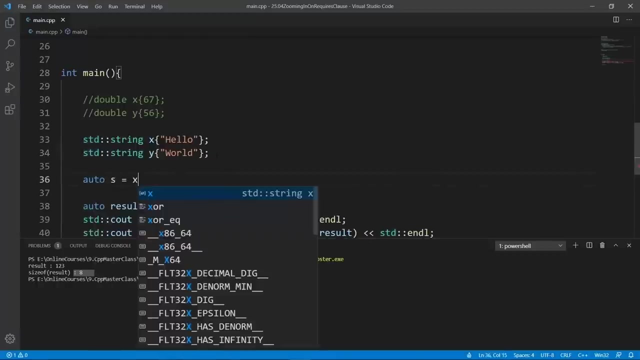 and at the moment we do this. you see that we have a problem. why do we have a problem? because it is now a requirement for the result of a and b to be convertible to add. remember that you can add up two strengths. for example, you can say auto s and say x plus y. 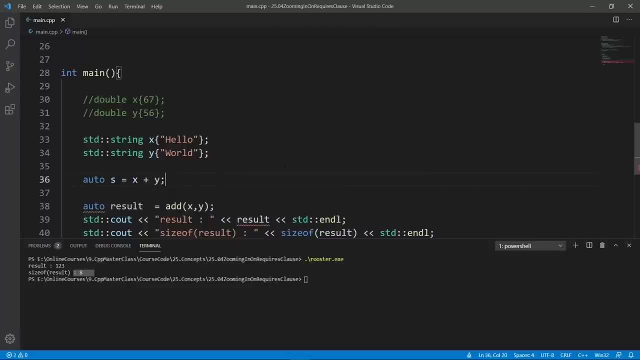 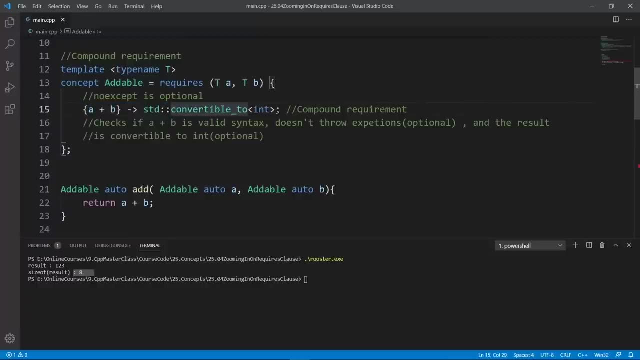 this is going to work because you can add up two strings and this is going to concatenate them, so this is valid syntax. why are we failing here? because we have a requirement for this to be convertible to an end, and the strength isn't really convertible to an end, so this is going to fail. 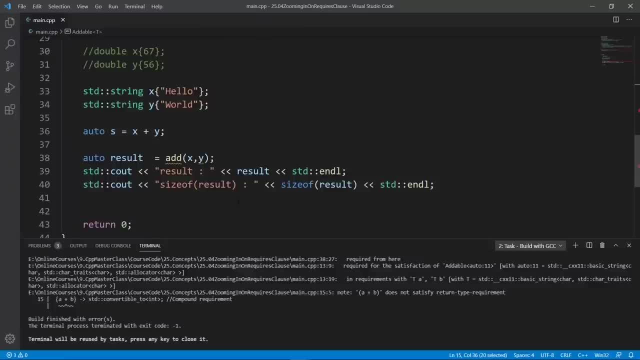 let's build this program and show you that this is actually the case. we're going to see both finished with arrows and let's see the error we have. okay, so constraints not satisfied. it's going to say required the satisfaction of addable, with auto here in requirement, and it's going to say a plus. 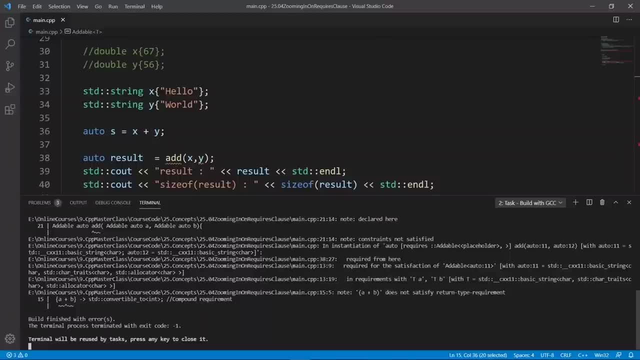 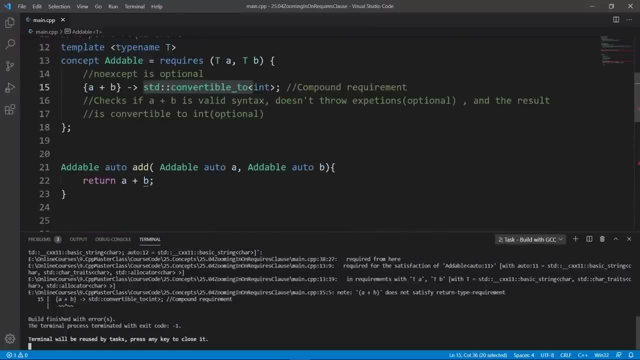 b does not satisfy the type requirement because what we get after adding a and b is not convertible to a net. and you see that here a plus b convertible to a net. this is going to fail. okay, so let's try and remove this requirement to convert to ant and see that this actually works. we're. 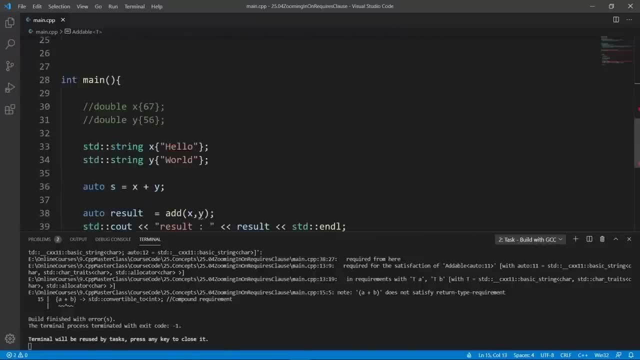 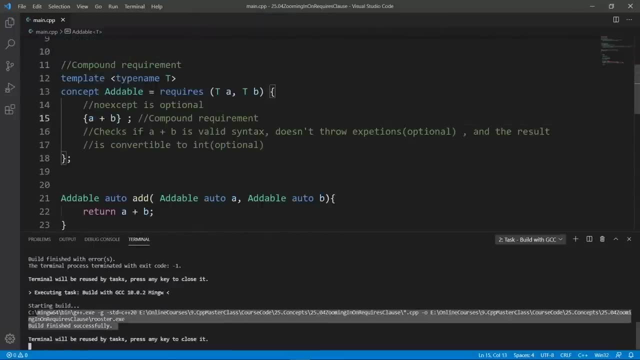 going to remove this. i'm going to cut this out and try to build again. i am going to use gcc to world- and now you see that this is welding, because we no longer have the requirement of the return value of this expression or resort. i should say. 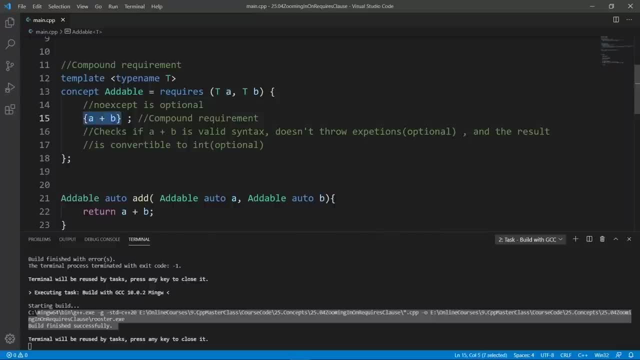 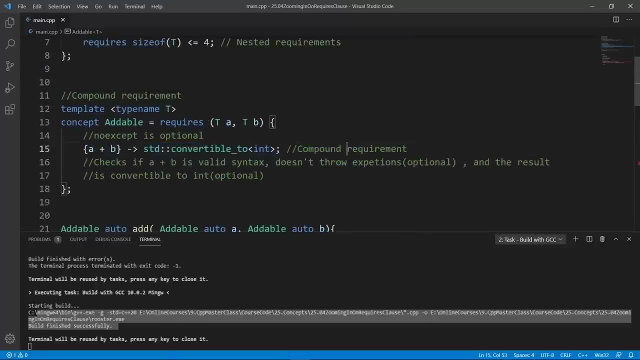 the result of this function now doesn't have to be convertible to an. okay, let's put this back, because i want you to see this later as a reference. and now you know how you can use compound requirements to really put constraints on your function templates. this is really all we. 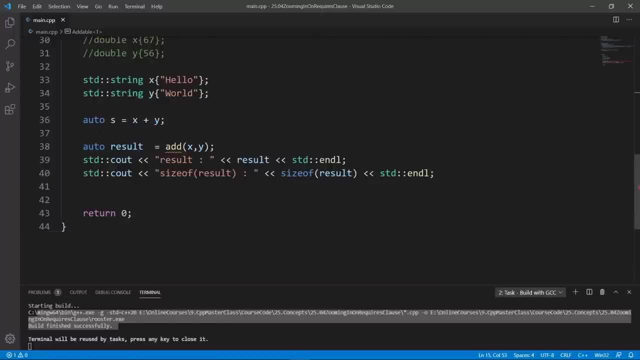 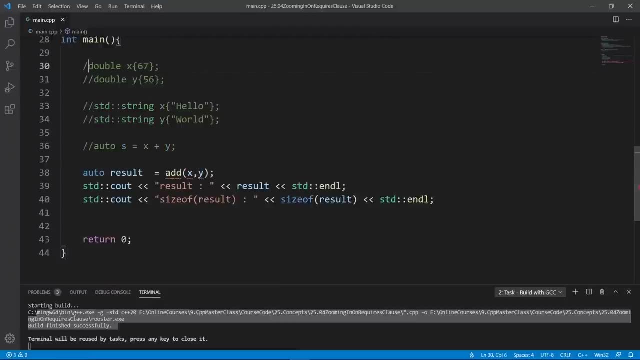 set out to do in this lecture. i hope you found it interesting. i think i should comment out these guys, because i don't like to leave you with code that has compiler errors. let's turn this back to double so that this works. we're going to weld again. okay, the world is good and we are going 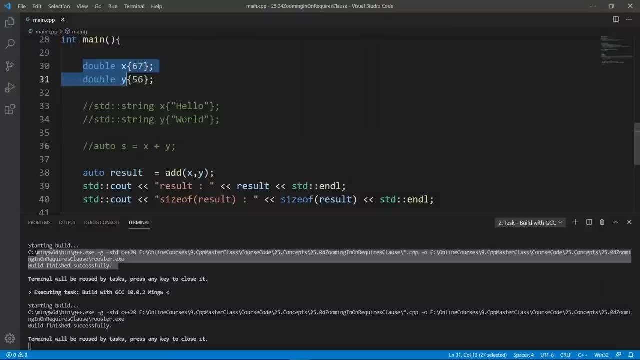 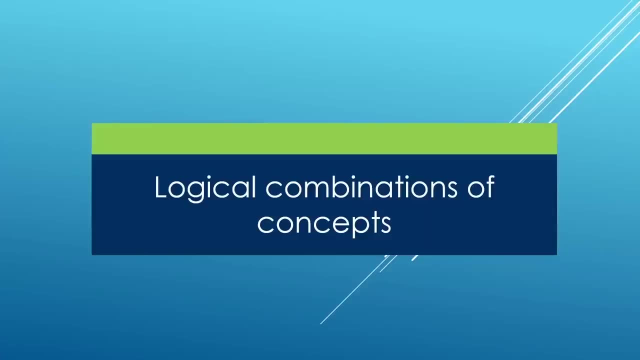 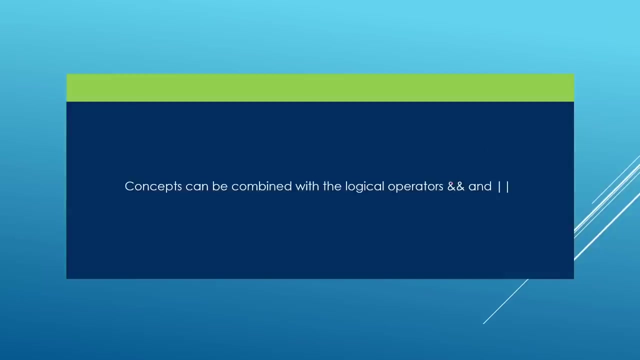 to stop here in this lecture. in the next one we're going to see how we can combine concepts and do some crazy things. go ahead and finish up here and meet me there. in this lecture we're going to see how we can combine concepts using logical operators. we can combine concepts using the. 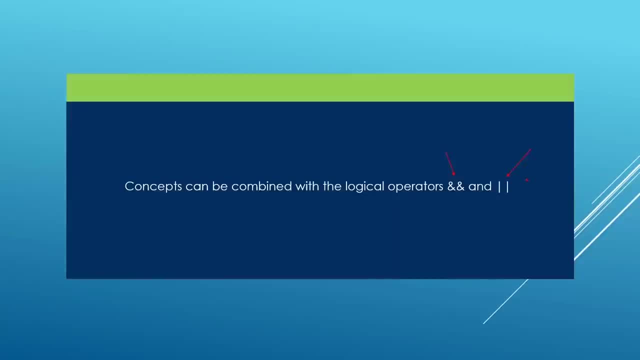 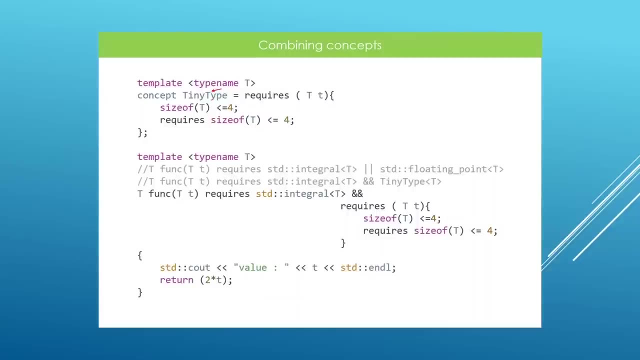 and operators operator and the r operator, as you see here. let's look at a simple example. here we have a concept. it is tiny type we have seen before- and it's going to check that the size of the template parameter we pass is less than 4.. it's going to enforce the syntax with a simple requirement. 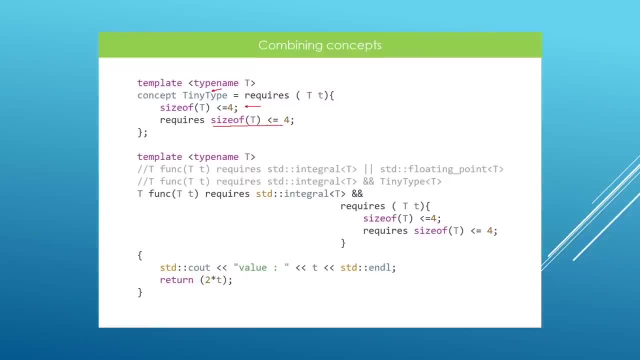 but it's also going to enforce for the value of this expression to be true. if the value is not true, the concept is going to fail, and we are using a nested requirement for this. so this is what we're going to do in this lecture: we're going to see how we can combine concepts and do some crazy things. 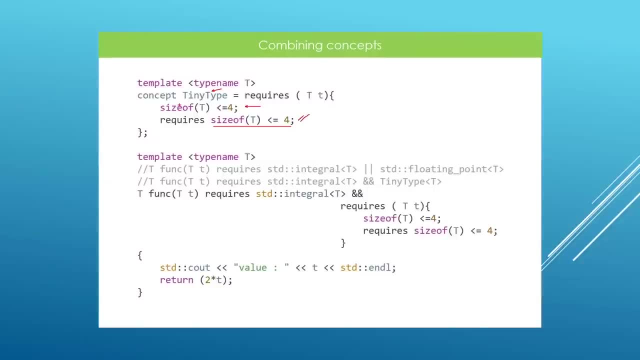 concept. here let's try and set up a function and see how we can combine this concept with other concepts. here we have a function. it is going to return a t, the name of the function is funk, it is taking in our parameter and here we have the body of the function within. 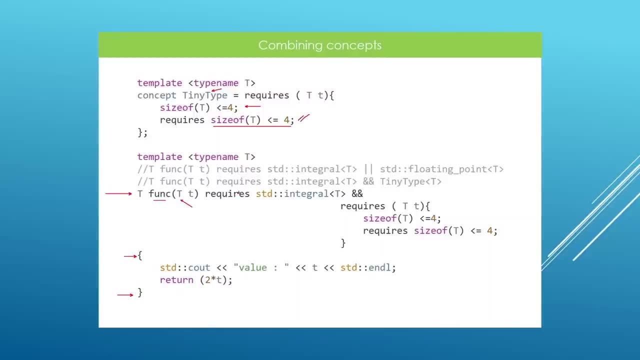 these two curly braces. but what we have here is a concept we want to apply to this function here, and the first line here is going to show that we can combine a concept like we do here. so this entire thing is going to be a logical combination of concepts, so we can require that. 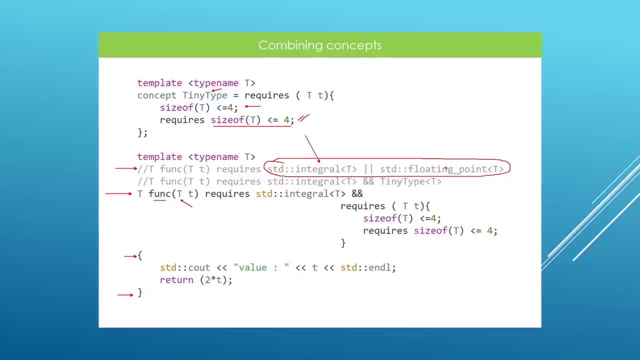 the template parameter be either an integral type or a floating point type, using the or operator here. another thing we can do is use the and operator, as you see down here in this second line, and we're going to require that the template parameter is both integral and a tiny type. 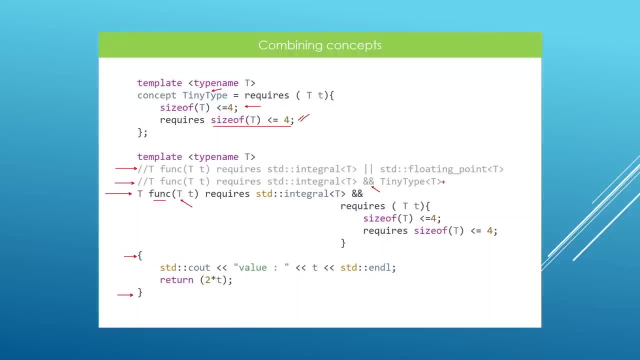 and the compiler is going to enforce these things, as we are about to see in a minute, when we hit visual studio code, you can even specify your concepts in place. for example, the third line here is going to say: we require for the concept to be integral, so it should be an integral type, and we're going to specify our tiny type concept. 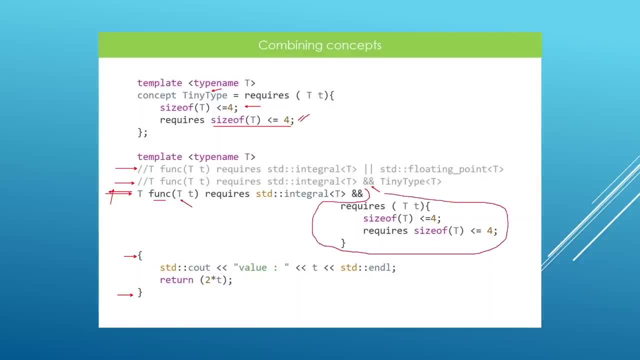 in place. you see, we are doing that right here in the function declaration and this is going to work. this is a valid c plus plus syntax, but i don't recommend this because this is going to make your function declarations really ugly. so now that you know this, we're going to head. 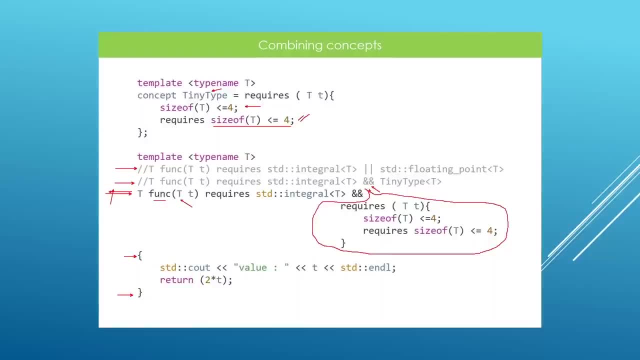 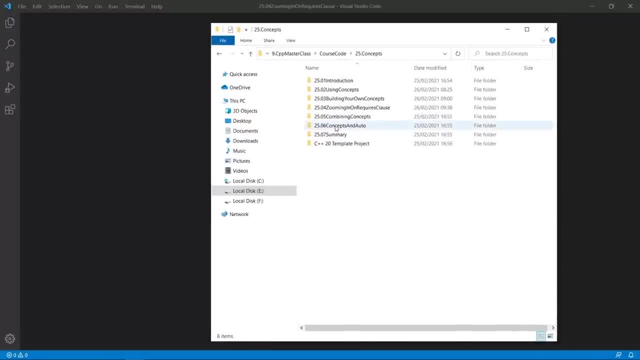 over to visual studio code and play with this a little more. it's just using the or and and operator to combine concepts. okay, here we are in our working folder. the current project is combining concepts. we're going to grab our template files pretty quick and put them in place, and we're going to 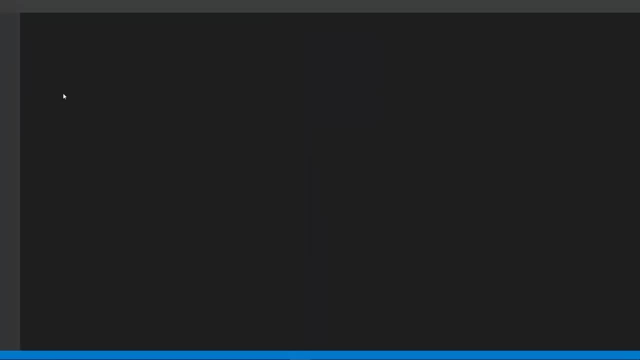 open this in visual studio code, as we always do, by dragging and dropping. here we have our file. we're going to open that file and we're going to drag and drop it. here we have our file. we're going to open the up and close the left pane here. i don't like it- and we're going to include our concepts library. 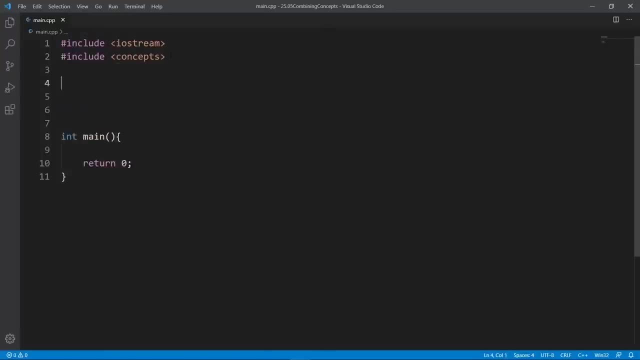 let's do that. we have this n. the first thing we're going to do is to put in our tiny type concept here. so it is tiny type. it's going to require that the syntax for size of t less than 4 be supported. this is a simple requirement, again, and we're going to require that this expression be true. 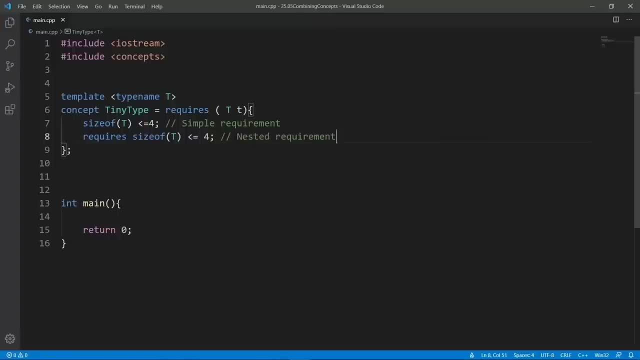 and we're doing this using an s- that requirement. okay, now that we have this concept, we can combine this with other concepts. let's use the same function we've been using all along. so we're going to say template, type, name, team and we're going to put in our requires clause. so we're. 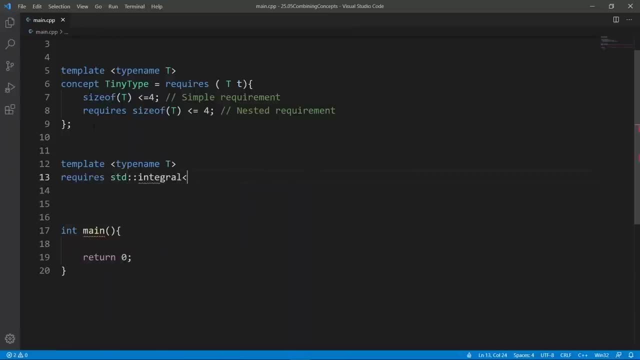 going to say requires: we can use std integral and say t and say: or it should be std floating point. i think we have this and this is a concept we have which is built into the c++ standard library. we can use this. now that we have this, we can then say the signature of our function t and it's going. 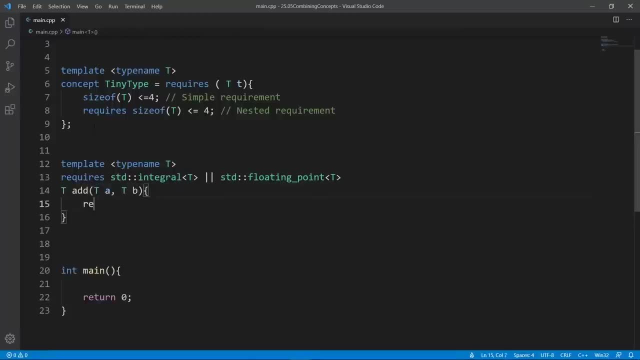 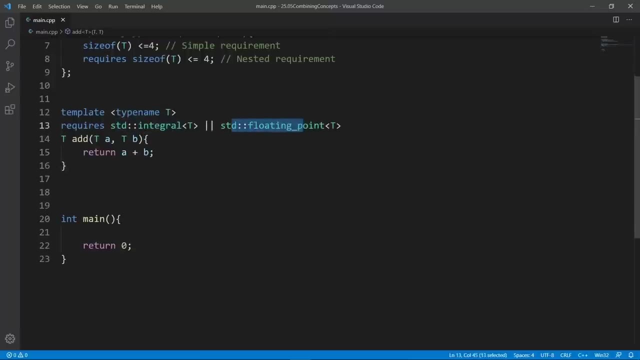 to add up t a and t b and it's going to return the sum of a and b. now you can only call this function with either integers or floating points. if you try to deviate from this, the concept is going to fail and we're going to get a compiler error. let's go down and try this out. we're going. 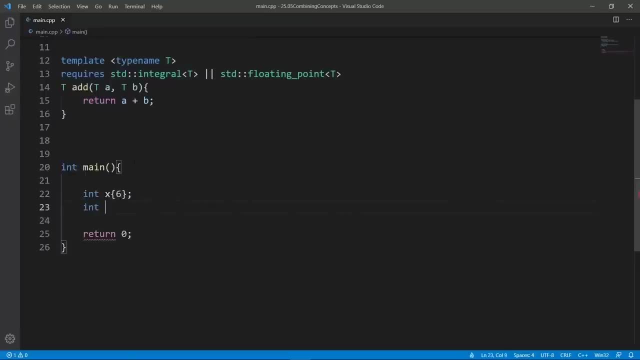 to say and x and put in a six, for example, and into y and put in a four, and we're going to add this up. we're going to say: add x and y. and if we do this, this is going to work, because this is an integer. 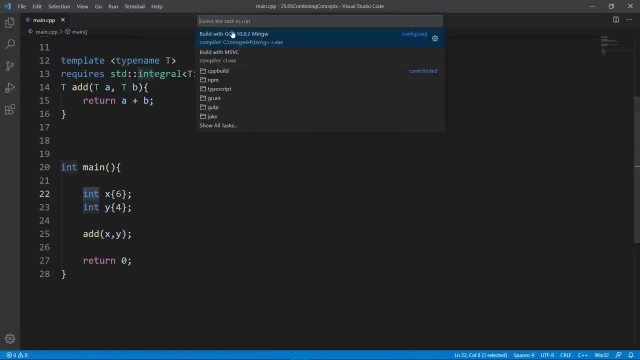 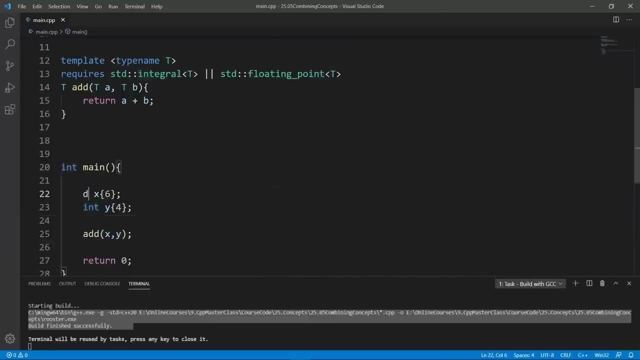 so the concept here is going to succeed. let's build with gcc and show you that the build is good. the build is good, so no problem, we can change this to double. it is going to work because double is a floating point. let's say double properly and if we build again, the build is going to go. 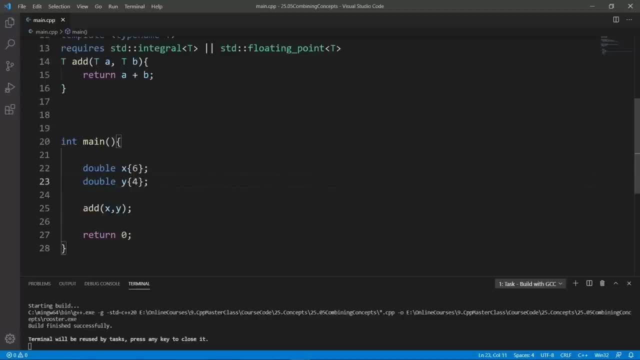 through. but if we try and use, for example, a string, let's say std string, string, that's a string and we're going to change this into double quotes. we can do that and say std string and put this in quotes- again, double quotes. okay, if we do this, you see we have a squiggly line. 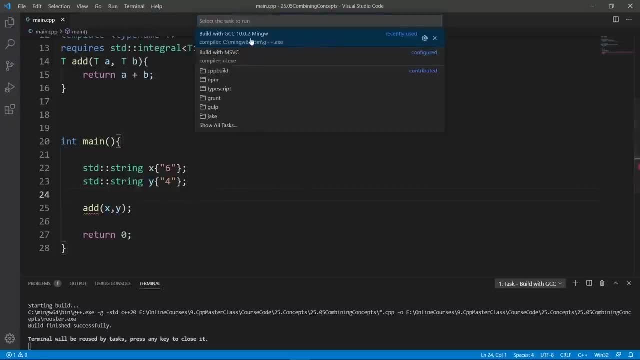 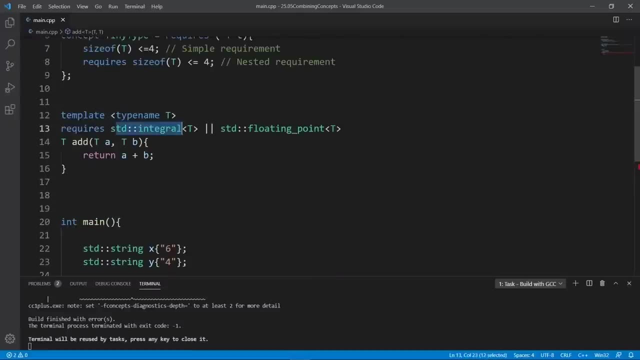 and if we're world, we're going to have violated our concept because the parameters that we pass don't satisfy this concept. it's neither an integral type or a floating point type- and if we go up here, we're going to see that we have violated our concept. and if we go up here, we're. 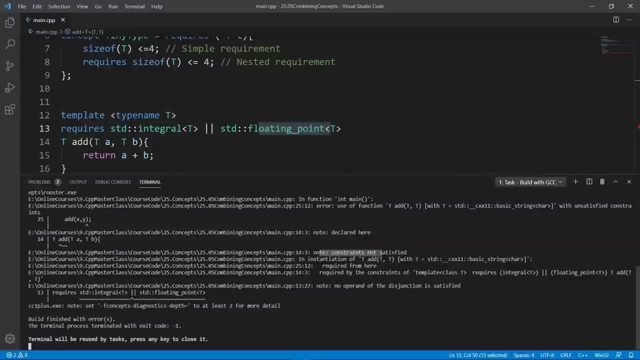 going to see that we have violated our concept. and if we go up here, we're going to see that we have violated our concept. and if we go up here, we're going to see that we have violated a concept constraint not satisfied, and it's going to say the concept that was not satisfied here, which is: 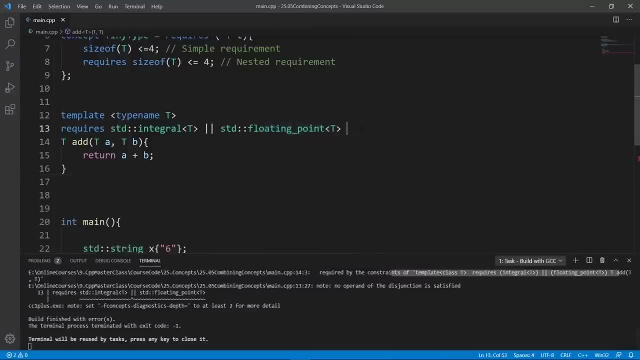 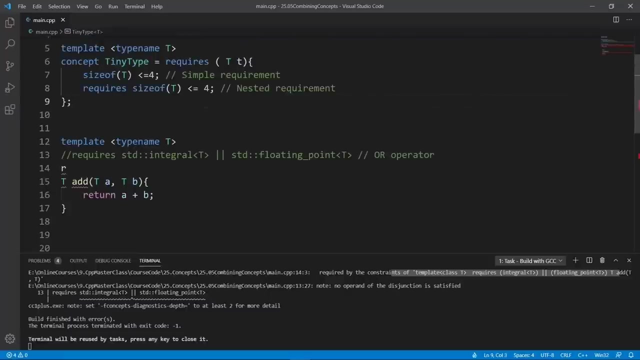 right here. okay, you can combine the two concepts using the or operator, but we can also use the and operator. let's go down and try and put up a simple example that is going to do that. now, what we're going to require for people to use this function is to satisfy both tiny type. 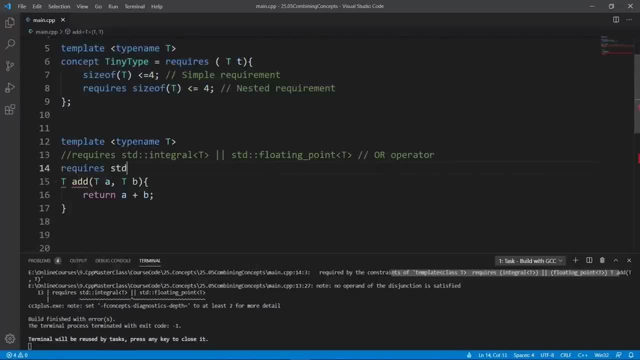 and integral. so we're going to say: requires s, dd, integral. i think we have this n and we're going to say and tiny time, and we're going to say our template parameter here the moment we do this, and let's turn this back to being ant, let's. 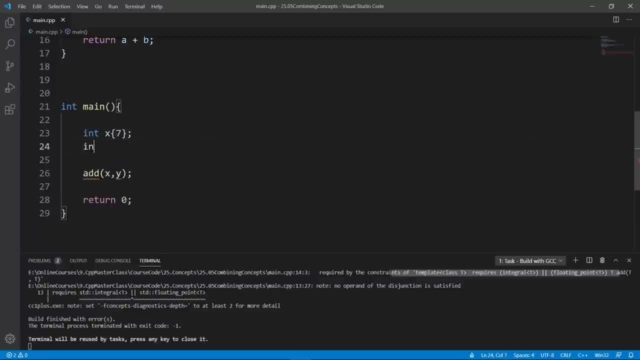 say ant x and put in a 7- what we had before- and ant y and say 4 or a 5, doesn't matter. if we do this, let's see our thing again. so tiny type requires for the size to be less or equal to 4. 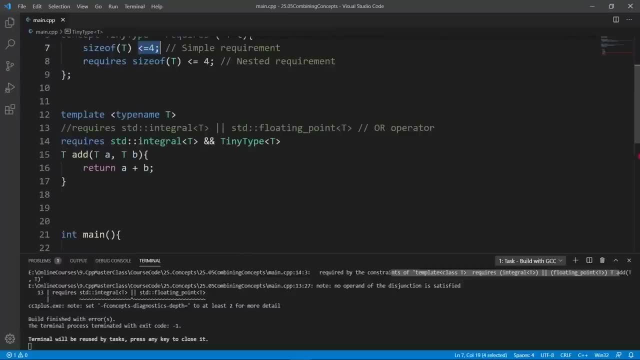 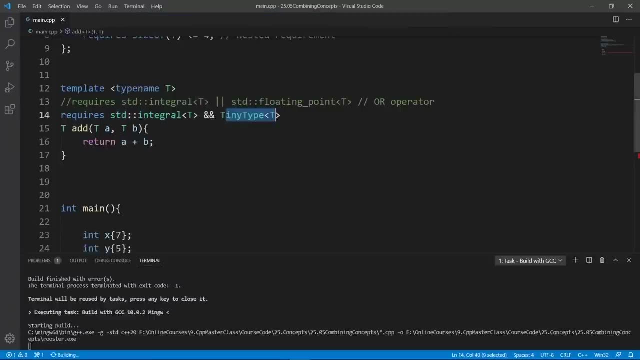 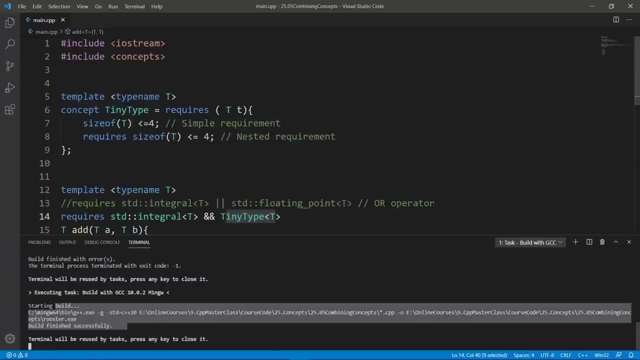 so ant is going to work. this is going to build because the concept is going to be satisfied. it is both integral and tiny type. let's build and see this run. you see, the both is good. our concept is satisfied, but the moment we try and use something that is greater than 4, we're going. 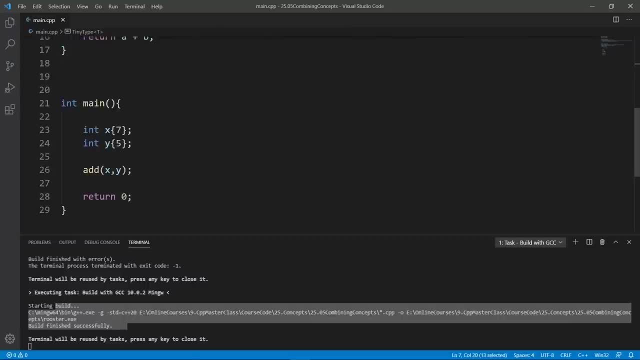 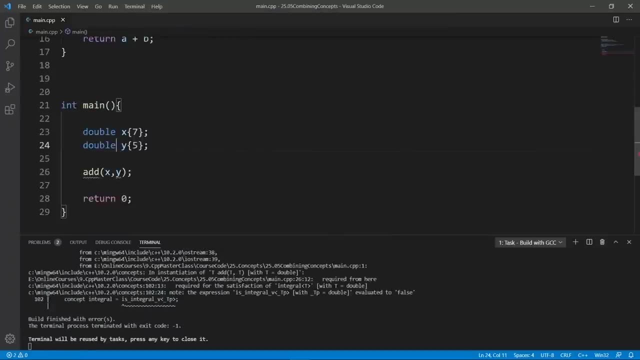 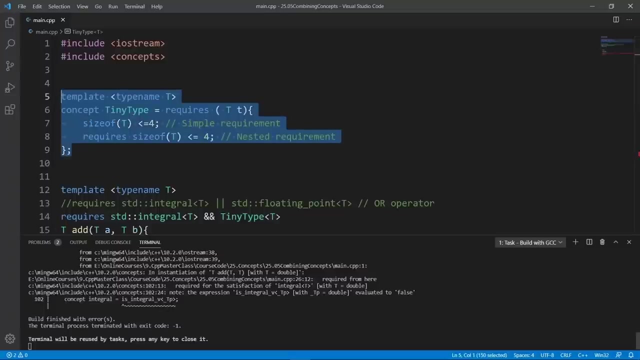 to have a problem. let's use a double, for example. we're going to change this to double and world. we expect compilation to fail because the type which is double doesn't satisfy the tiny type concept and we're going to see that here. okay, so we're going to see both finished with arrows and we're going to have a lengthy 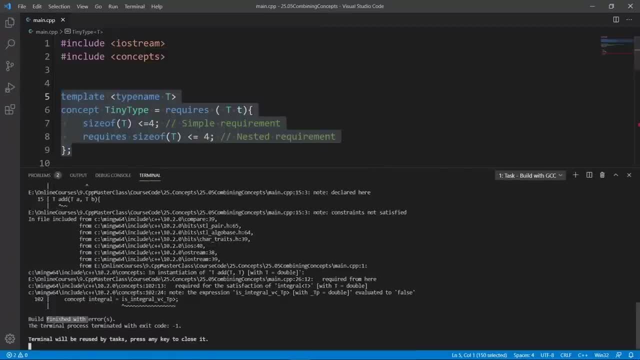 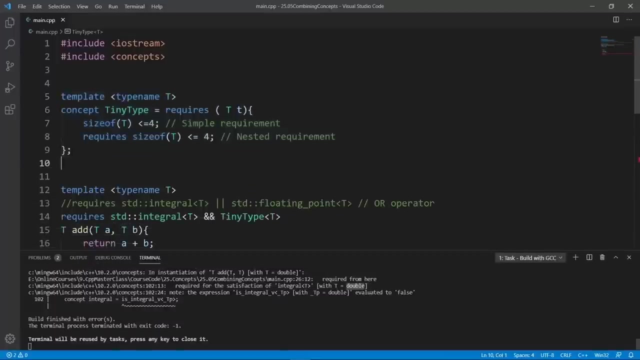 arrow here. but the meat of this is that we have a constraint which is not satisfied and it is that for required for the satisfaction of std integral. so double is not going to satisfy this. i think double was a really bad example because it's not integral, so integral is going to fail. what if we pass in long ant? okay, 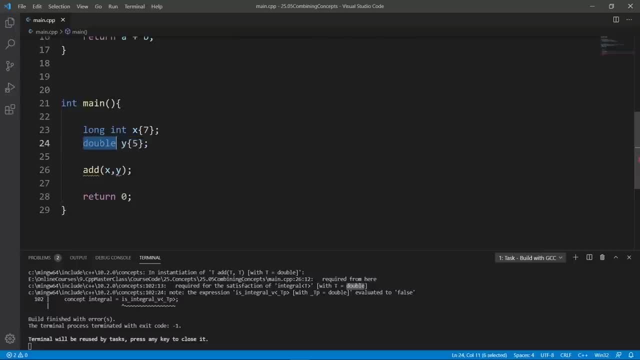 which is really an integral type, but it's not going to satisfy tiny type. so let's say long ant and we're going to build. now we are going to violate. let's use long, long ant because i think long ant is not large enough. so we're going to build, now we're going to fail because tiny type. 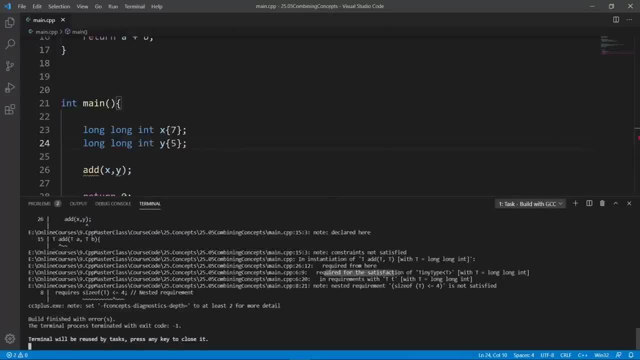 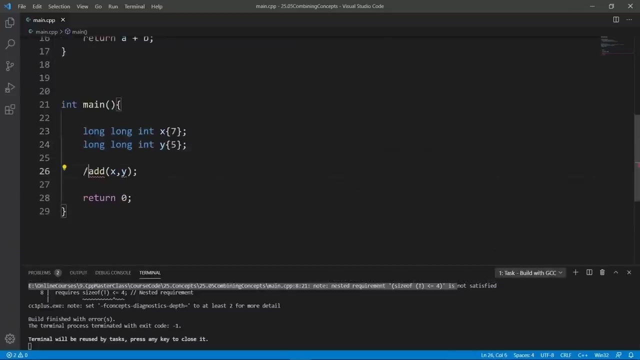 is not satisfied. you see, required for the satisfaction of tiny type, and it's going to say size of t is less than four, is not satisfied because, guess what? the size of long, long ant is greater than four. you can try and prove that by taking out this guy here and saying std c out. 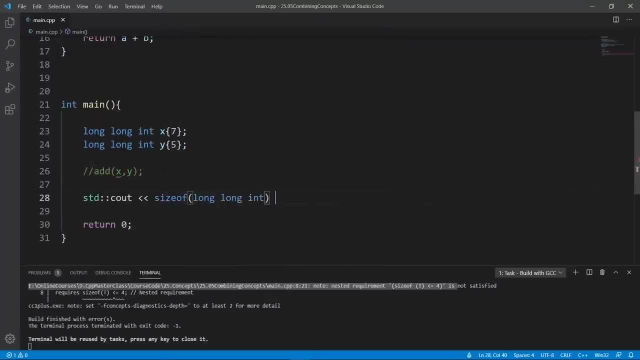 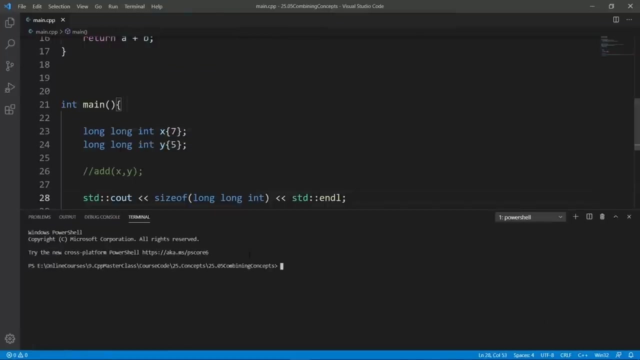 size of long long ant. we're going to see this print out and if we build now, we're not going to violate our concepts because we're not calling the function. the world is going to be good. what we want to do is run the program and see the size of long long ant. we can do this. rooster eight. the size of long long ant is eight. 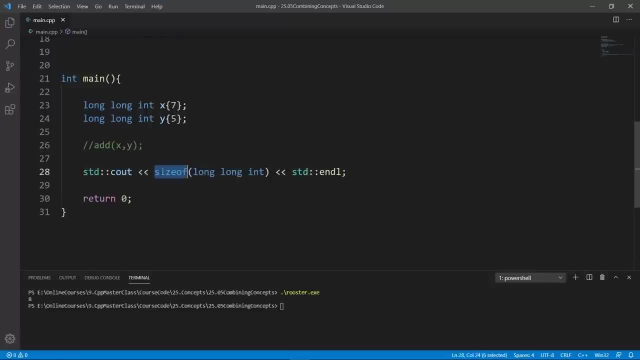 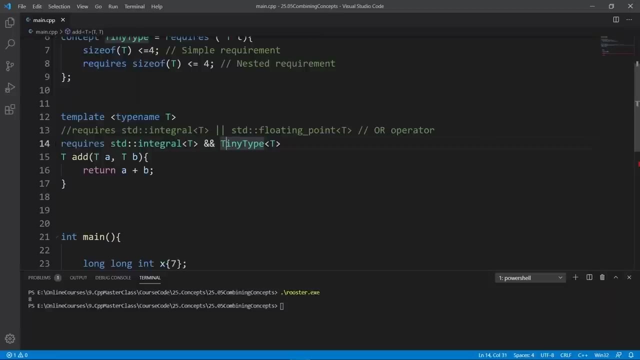 and it is going to violate our tiny type concept. okay, you can do things like this and combine the concepts, but we can even put our concepts in place. we can do something crazy and, for example, say let's copy this and we're going to go down and say: requires integral, but we're going to put 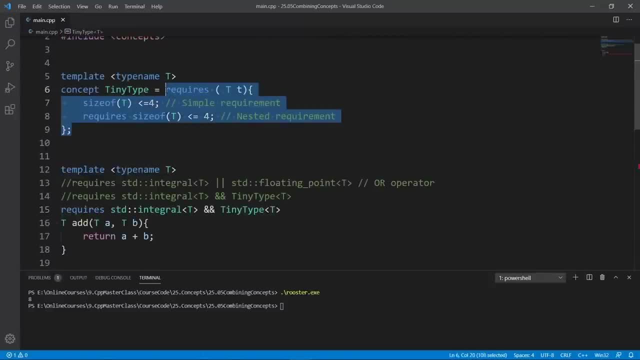 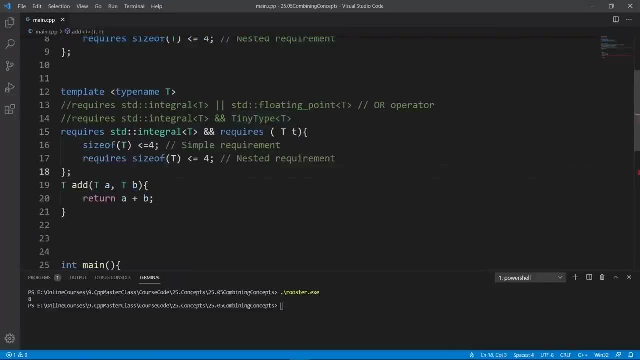 tiny type in place. for example, we're going to grab the requires close here and copy it and put that in place of tiny type here. we're going to do this and you're going to see that this is going to be valid c++ syntax if we take out the semicolon because it shouldn't be there. 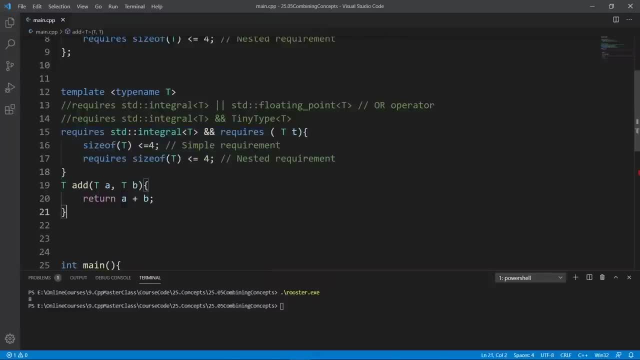 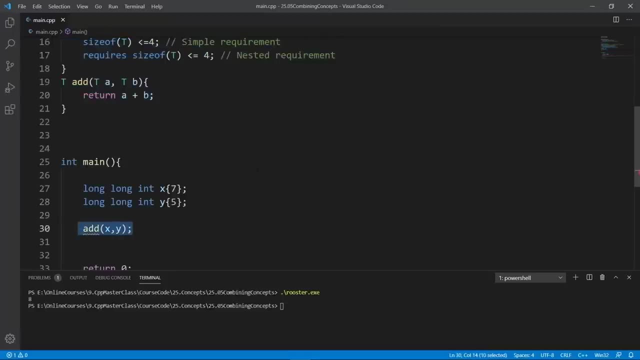 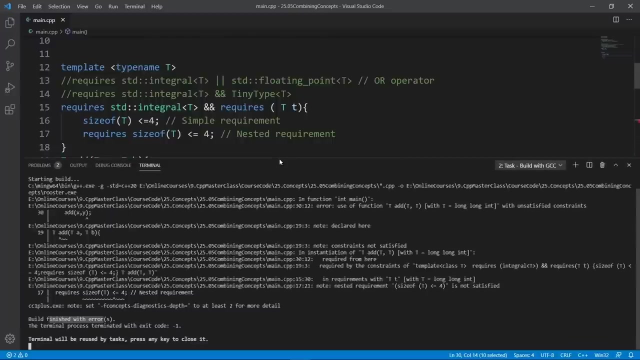 but look at this. this is really ugly. this is going to make your functions really hard to read, but it is going to work exactly the same way it did. if we call this function, we're going to violate tiny type. let's do that. we're going to build with gcc. we have an error. let's bring this up so that we can see what is. 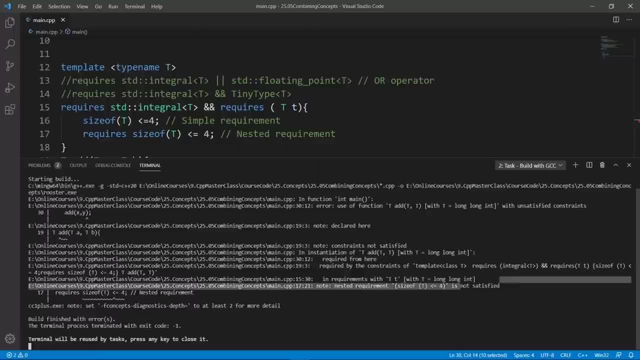 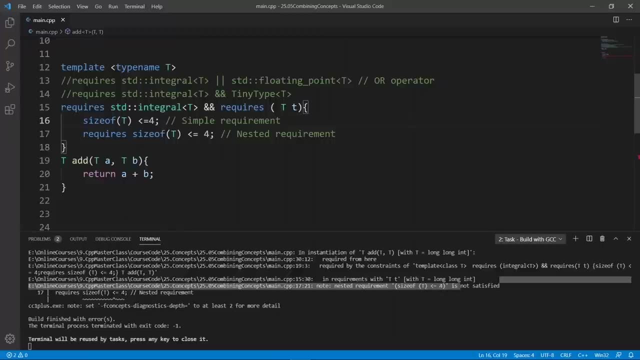 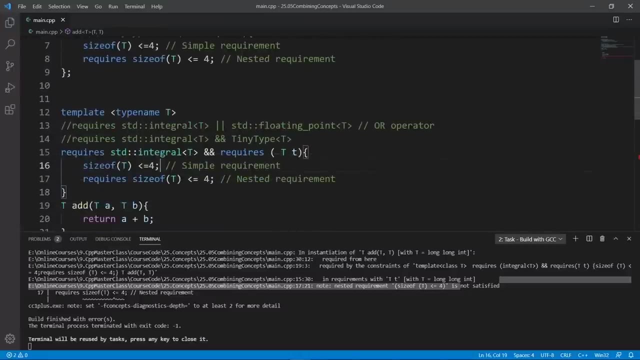 wrong. nested requirement size of t is not satisfied. this is a syntax you can use, but i don't really recommend this because this is going to make your code hard to read, and this is really all we set out to do in this lecture: looking at how we can combine our concepts using the and operator, and. 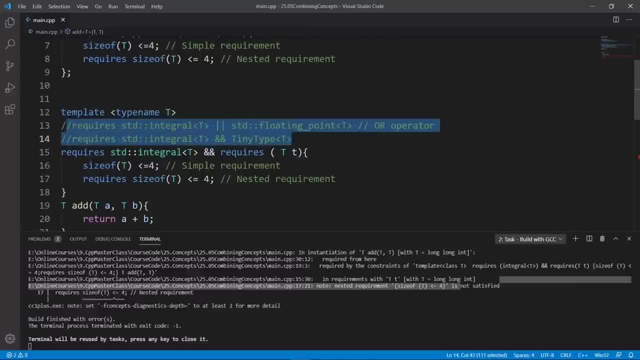 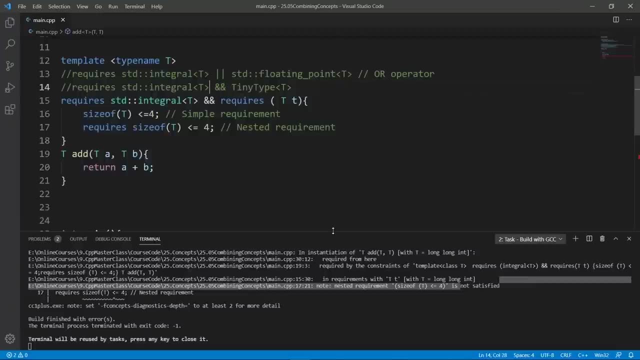 the or operator, and you can really use this in all the syntaxes for concepts we have seen. but i just used this in this lecture because it is simpler to show. we are going to stop here in this lecture. the next one we're going to look at concepts. 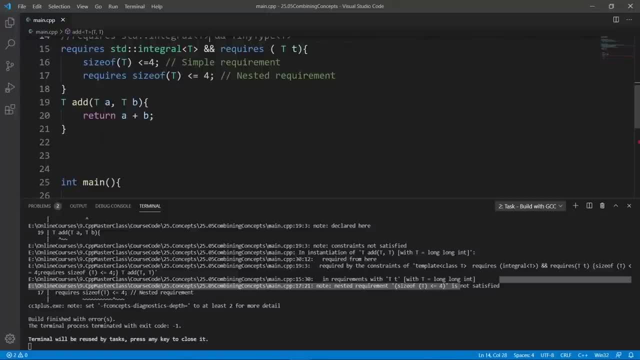 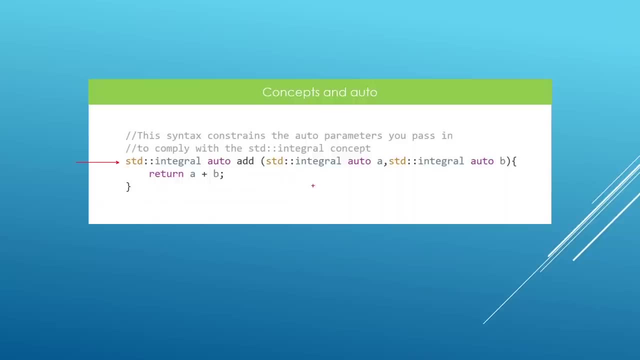 and auto. go ahead and finish up here and meet me there. in this lecture we're going to zoom in on concepts and the auto keyword. we have already seen that we can do something like this: we use the auto keywords with our functions and let the compiler generate our function template. 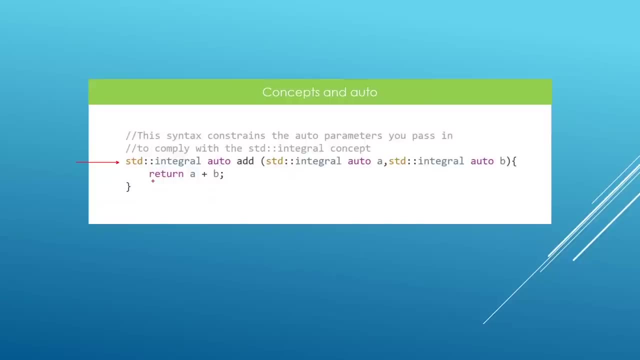 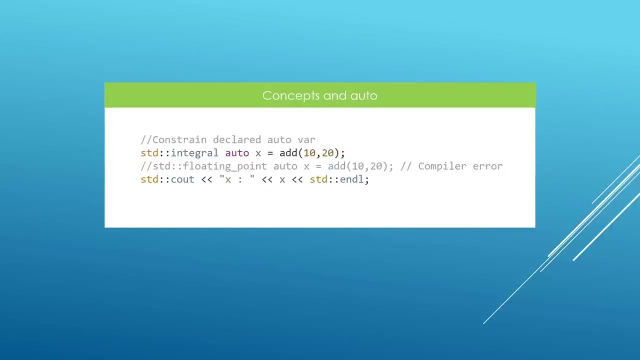 behind the scenes and this worked pretty well. we could had used syntax to put constraints on our other keywords and we saw that the compiler could actually enforce this and throw a compiler error if our concept here is violated. what i haven't shown you is that you can even enforce concepts on variables that you declare. you can do something like this: set up: 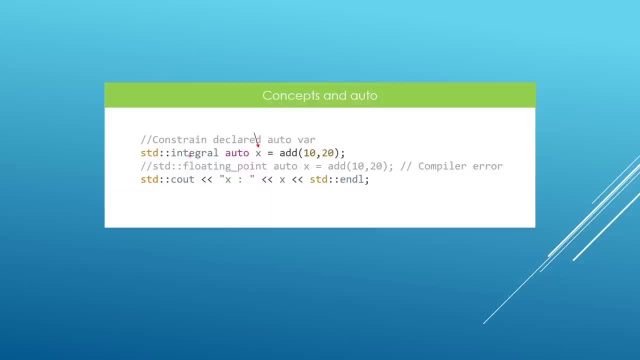 a variable, say auto x, and call the variable x and enforce for the variable to be an integral type. i don't really think you have much use for this, because once you call the function and assign a value to a variable, you already have an idea of what is going to come out of the function. 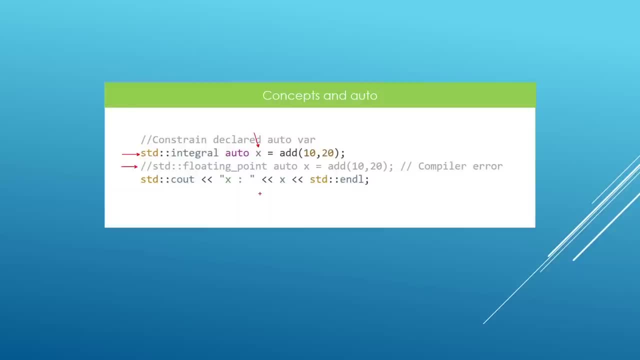 but if you have a use case for something like this, please go ahead and use this. it is going to enforce your concepts. you can even use concepts like this, set up a variable and assign a literal to the variable name using the auto keyword here. but i personally find this useless because 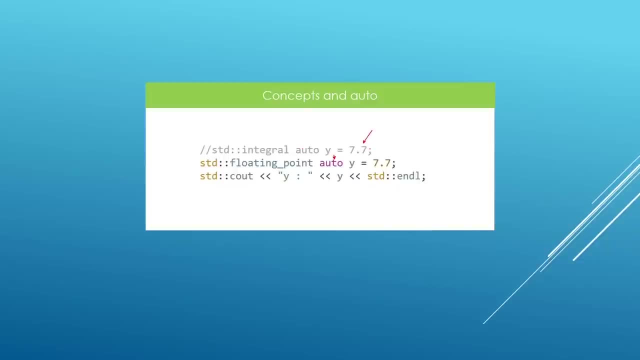 you are putting in the value yourself, why do you want to put a protection? if you know that you are putting in a double literal, then the variable should be of double type. i find this a little bit useless, but it is supported in c plus plus. if you have a use case for this, please go ahead and. 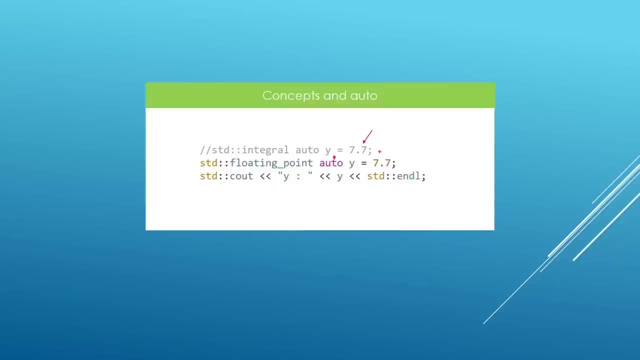 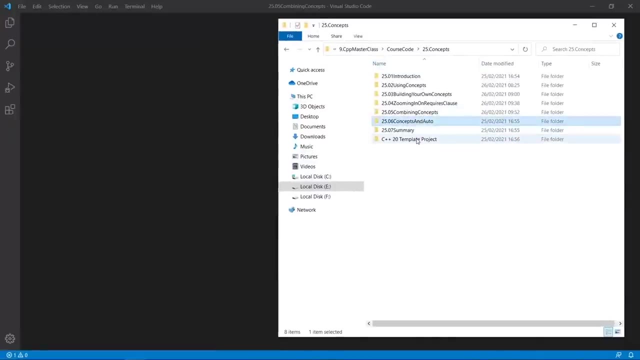 use this. now that you know this, we're going to head over to visual studio code and play with us a little more. okay, here we are, in our working folder. the current project is concepts and auto. we're going to grab our template files and we're going to put them in place and we're going to open this up in visual. 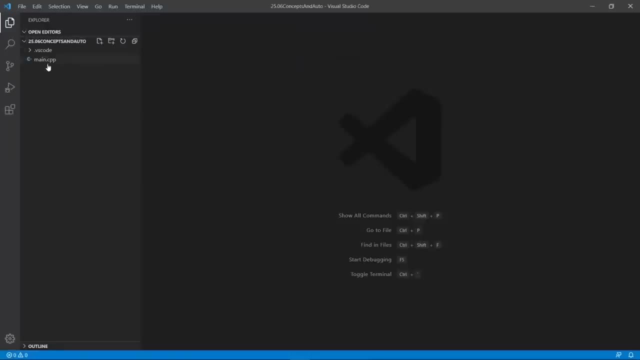 studio code. let's do that pretty quick. we're going to have our folder open, we're going to open the main cpp file, close the left pane and clean things up a little bit, and we're going to include our concepts library and we're going to put in our function, which is going to be using the auto. 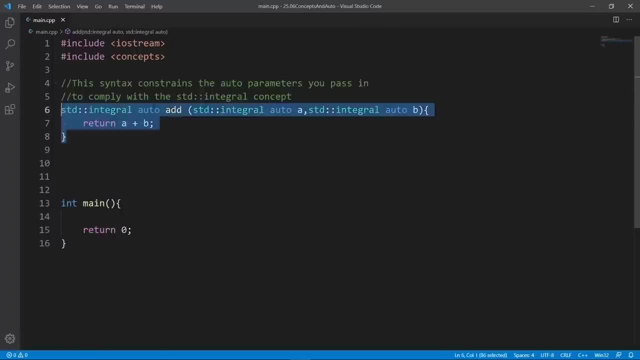 keywords to really make the syntax nice and cool. but we're going to be constraining our auto parameters here to use integral types. if we call this function with something that is not an integer or an integral type, really we're going to get a compiler error. so if we go down here, for example, and say: 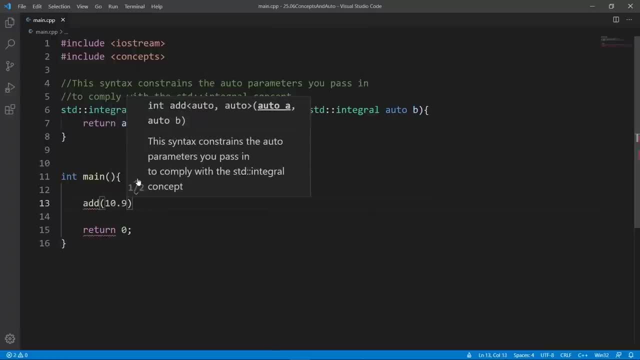 add and say 10.9 and 0.1, we're going to get a compiler error because 10.9 and 0.1 are double literals and we only support integral types in this function here. so let's go ahead and show you. 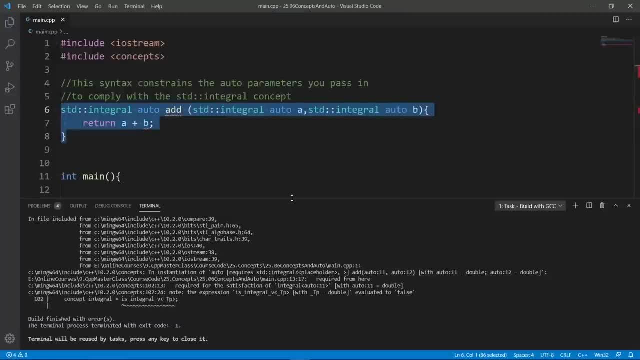 the error. but you must know this by now, because the function is going to be used for a lot of fields, because we have done this like a gazillion times. the concept integral is going to be violated and it's going to say required for the satisfaction of integral. so the concept is failing. here we're. 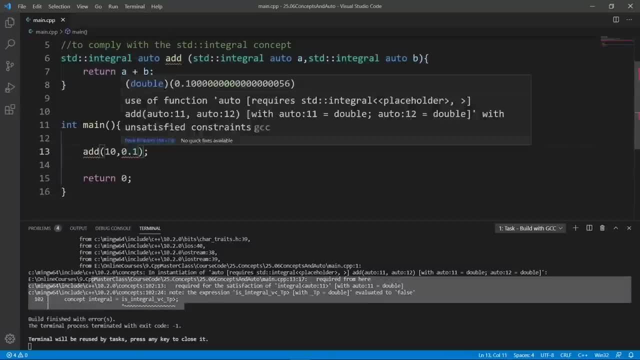 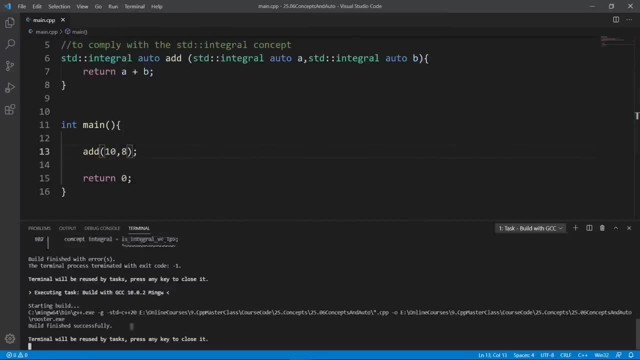 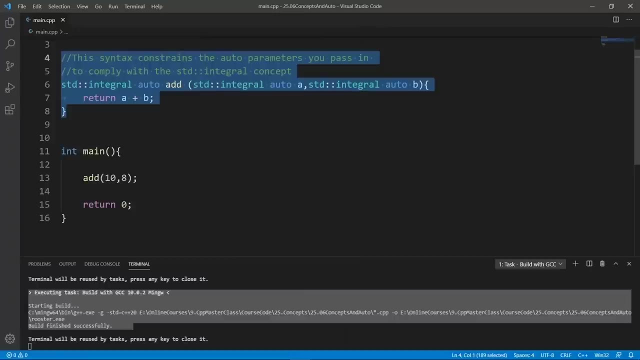 going to get a compiler error. but if we change this, for example, to 10 and 5, put in whatever you want which is an integer, this is going to work. we're going to build with gcc. you see, the word is good, so you can use auto with concepts like this. we have seen this syntax already a couple of times in. 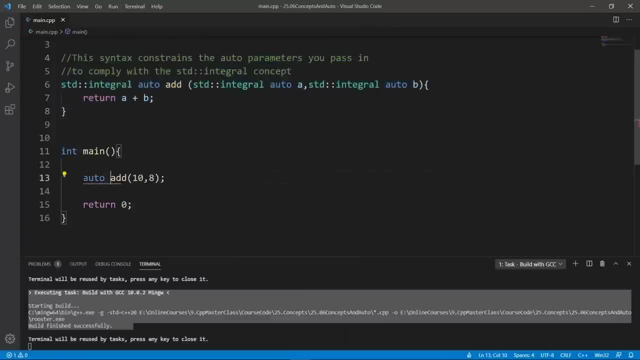 what we haven't seen is that, for example, you can set up a variable in main and call this x, y, naught and say this variable should satisfy the concept and specify the concept you want. for example, let's say std integral. and if you do something like this, let's see what we get from this we're going to. 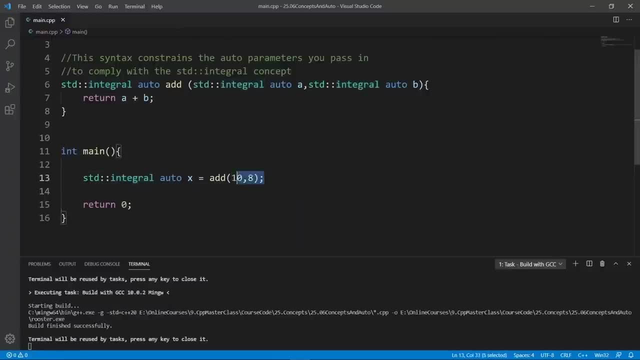 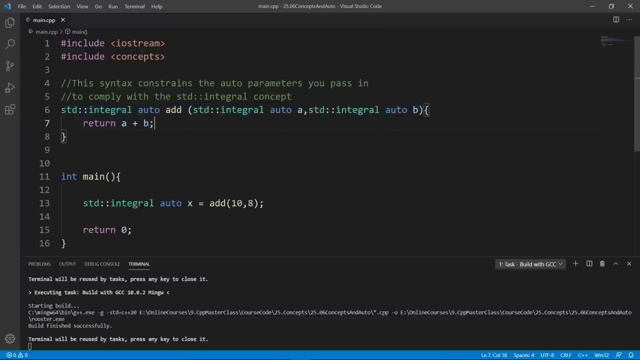 world. you see, the world is good because if we add up these guys, we're going to generate an integer instance for this function and we're going to deduce the return type as: and. so the return type is going to be integral and it's going to be assignable in our variable here. but if we change, 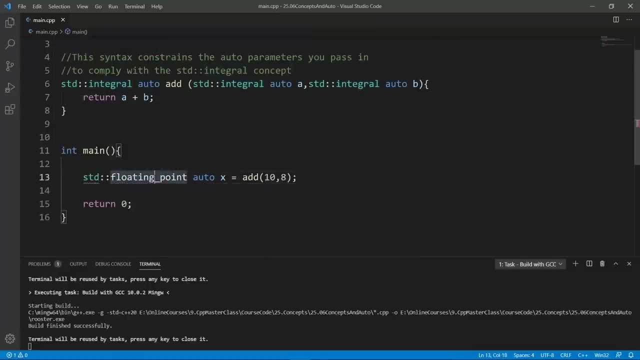 to floating point. i think we have this concept in place. yes, we do, but it is going to fail because what we get from this function is going to be an integer and we can't assign to this, because this concept here is saying: what you try to assign to this variable here should be a floating. 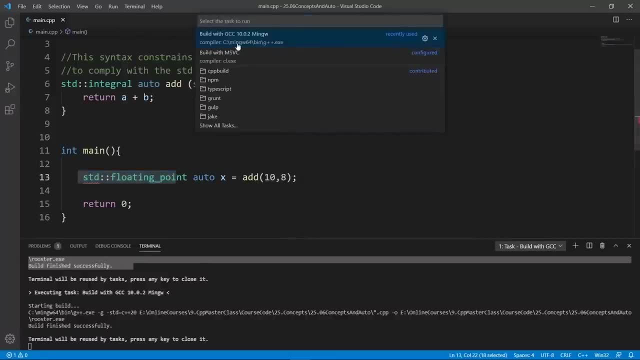 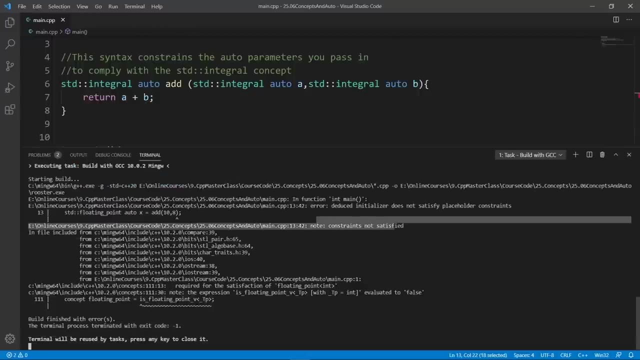 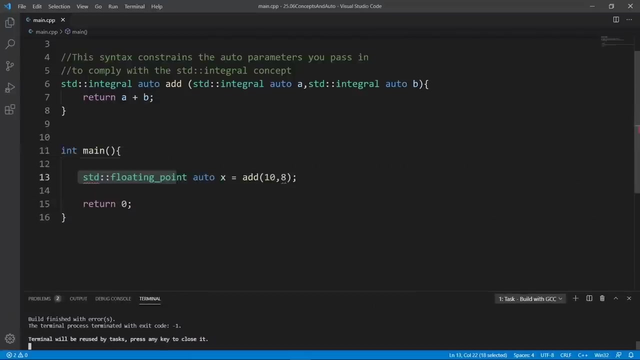 point. this is the meaning here, and if we do this we're going to get the error probably. so we have the error and it's going to say constraint not satisfied, and it is going to say the constraint we didn't satisfy, which is is floating point here. this is how you can put constraints on your. 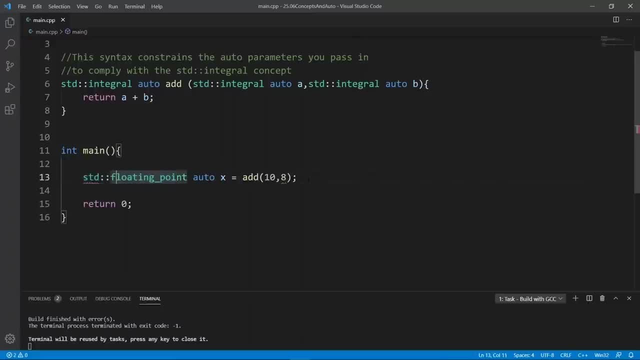 variables even when you are declaring them. so another thing we can try here is to assign a literal to this variable. here let's put in a 3.9 and see if this actually worlds and compiles. let's build with gcc. you see, the build is good. 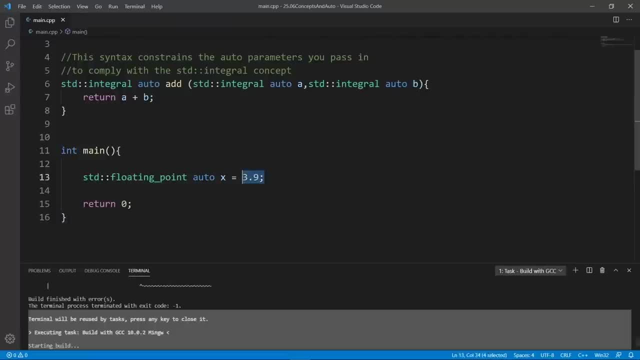 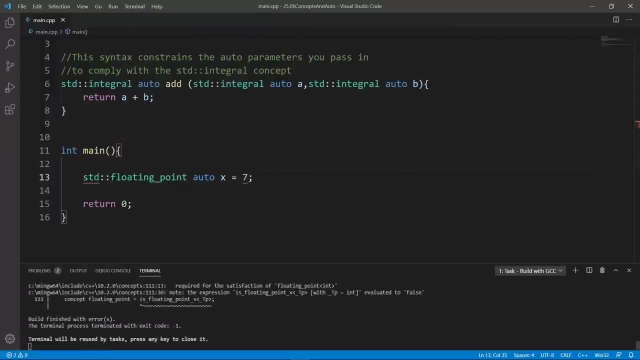 and the requirement is for what we assign to this variable here should be a double, and a 3.9 is already a double, so no problem. but if we try and make this seven, for example, this is going to fail, so let's build again. you see, the concept is going to fail and this is how you can use these. 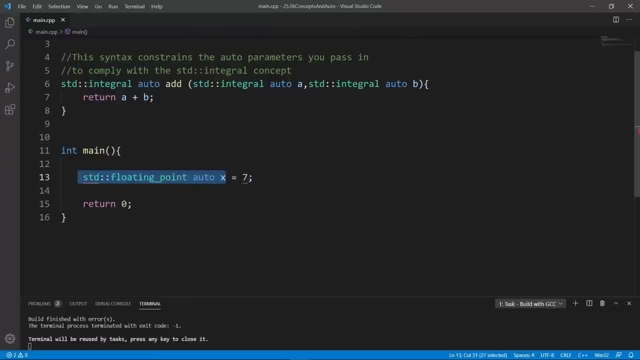 things to constrain the variable here. so let's build again and see if this actually works. so let's build again and see if this actually works. i personally find this a little bit useless, at least in this case here, because i know that i have an integer literal and i am assigning this to a variable. why do i need the help of concepts to? 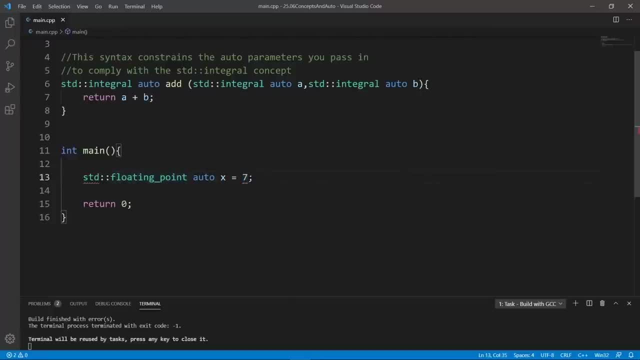 really constrain my variable here, but in the case where you are calling a function, for example using a five and an eight, this can come in handy because it's not easy to keep track of the return type you get from the return type of the function. so let's build again and see if this actually works. 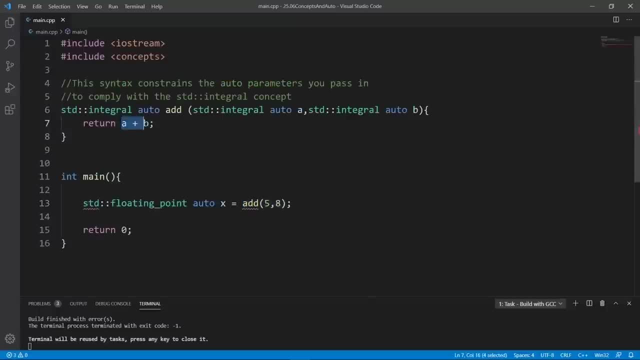 from a function because the function might have a return expression that has multiple different variables, and it's not easy to keep track of what you get back from a function, and you can use a constraint like this to make sure what you get from the function is what you want and if it's, 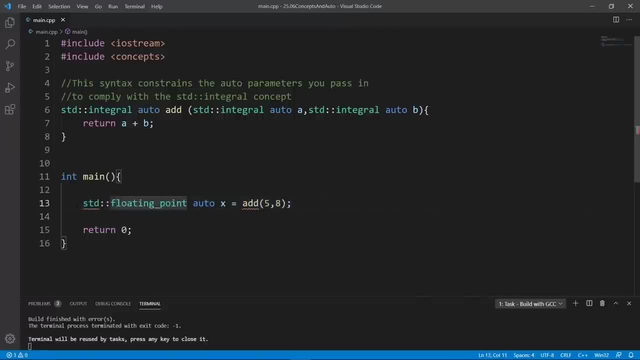 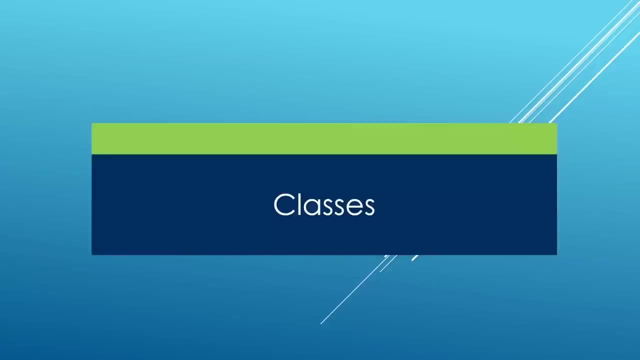 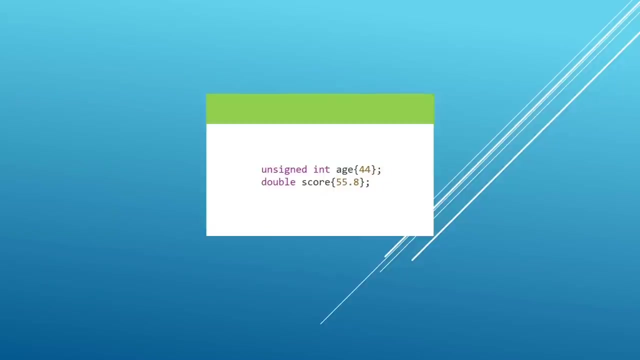 not what you want. you're going to throw a compiler error because the concept you used is going to fail. I would like to welcome you in this new chapter where we're going to be learning about classes. Classes are a mechanism we have in C++ to build our own types and use them like we have. 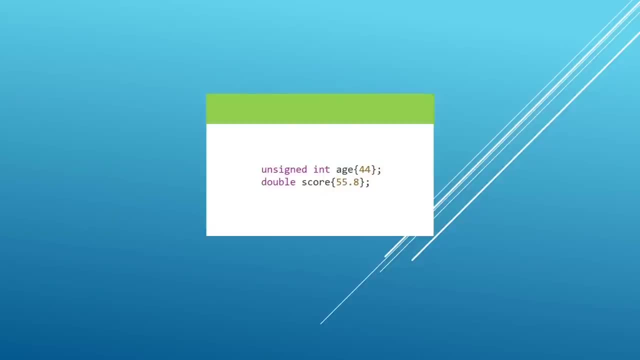 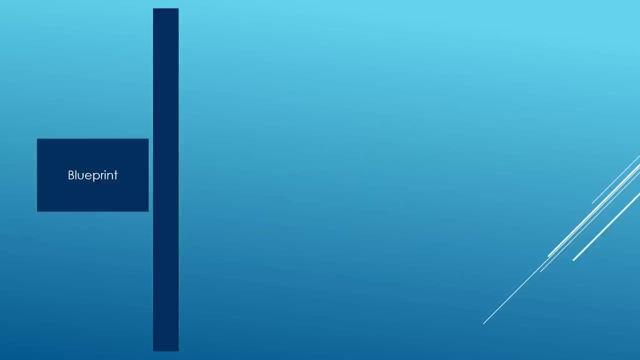 been using other built-in types like n to double or whatever, and we're going to be able to do that by setting up blueprints of our class types and we're going to be using those blueprints to build actual objects that we can use in our C++ program. So, for example, we can have a class as a blueprint. 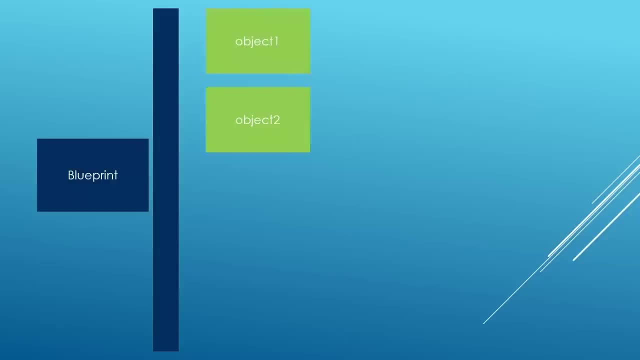 and we can create a class as a blueprint. and we can create a class as a blueprint and we can create real class objects in our C++ program as we need them, and we're going to be learning all about this in the next few chapters. We are going to head over in the next lecture and let you set up your. 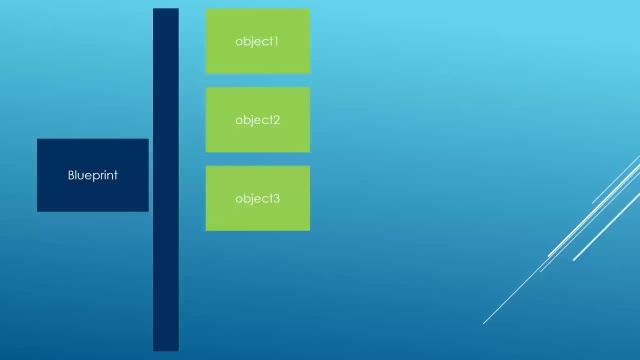 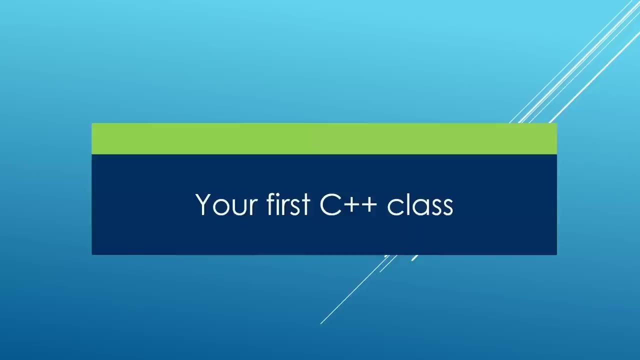 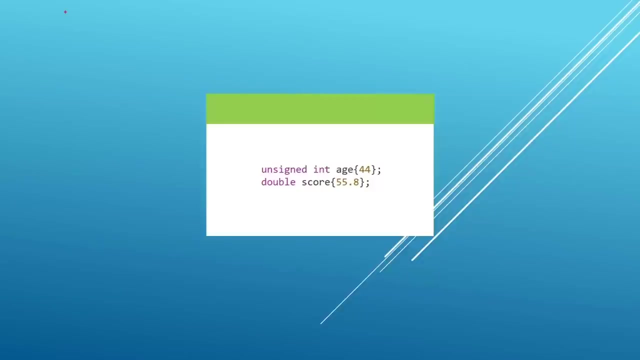 very first C++ class. Go ahead and finish up here and meet me there. In this lecture you are going to build your first C++ class. Classes are a mechanism we have in C++ to be able to build our own types. If you remember, so far in this course we have been using basic types like n and double, and we were 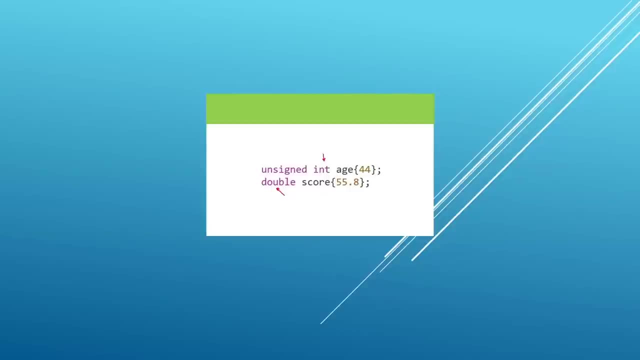 using them like this: We say the type of the variable, we give the name of the variable and then we initialize this variable and we can use this throughout our program. Now we are at a point where we need to start designing our own types. Suppose we want to build our own type that models: 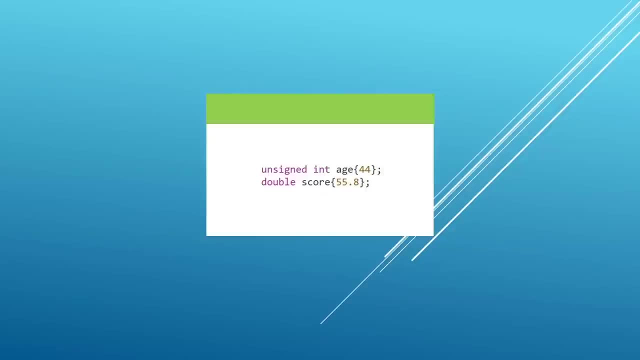 a person. for example, Suppose a person is a person, that is a person, that is a person. that is a person is defined by the name, the age and the address, And we want to model persons in our program and use them as players, for example. And when we have the properties of a person, we can do all kinds of crazy. 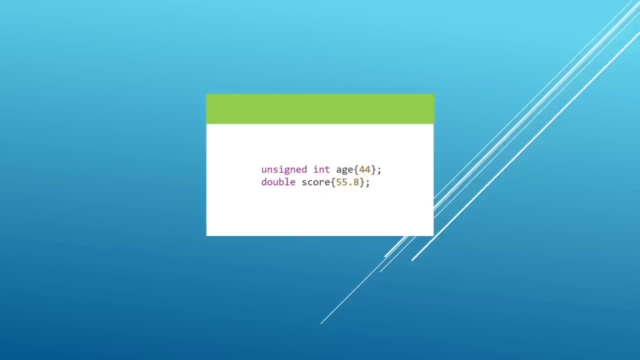 things with them. We can make them jump up, for example, if we are designing a game. We can make them run, We can make them fly. We can do all kinds of crazy things. In this lecture, we're going to use a cylinder as an example. And we're going to use a cylinder as an example And we're going 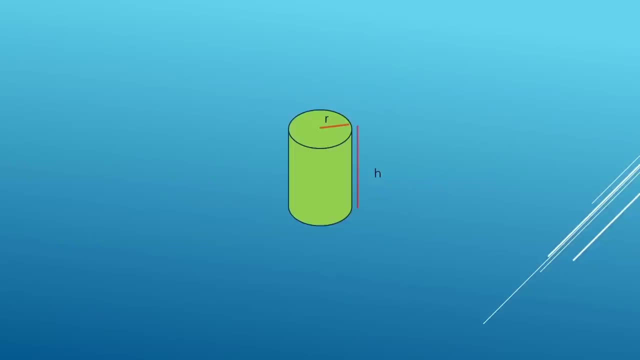 to model a cylinder in our C++ program. A cylinder is defined by two things: It has a base radius, which is modeled by this r you see here, And it has a height. And when we have this information about our cylinder, we can really do all kinds of crazy things. For example, we can compute its area. 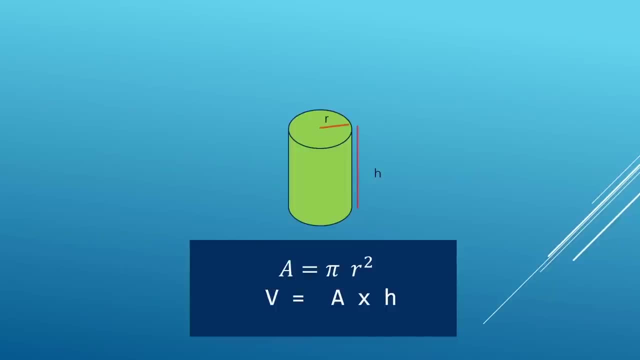 the base area And the formula to do that is pi r squared. This is a formula you get from your basic method And we're going to use it to model a cylinder in our C++ program And we're going to do all kinds of crazy things with the cylinder if we have this information. So we're going to use 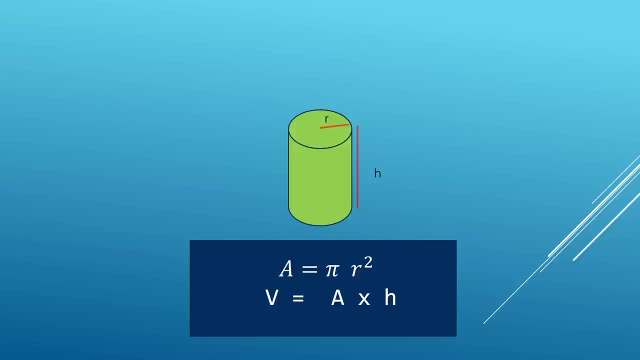 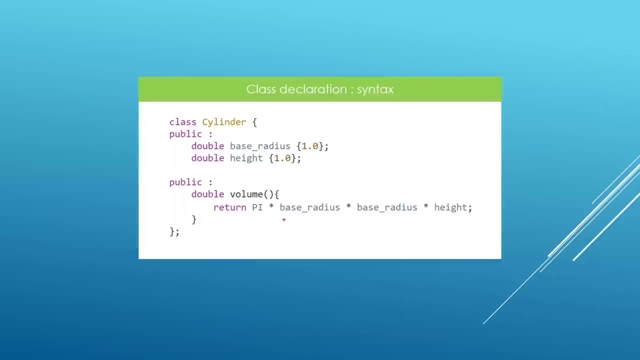 this information and model, a cylinder we can use in our C++ program, And we're going to be using classes to do that. The syntax to set up your class in C++ is really simple. You say class- this is the keyword you have to put in here. You say the name of your class. In this case it is: 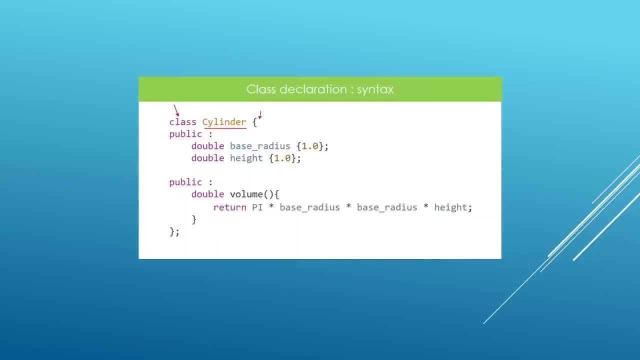 cylinder, as you see here, And then we put a pair of curly braces in place. The start is on top here and the end is down here, And after your class definition you're going to put a semicolon Inside the class. we really have two parts. We have member variables which are going to model. 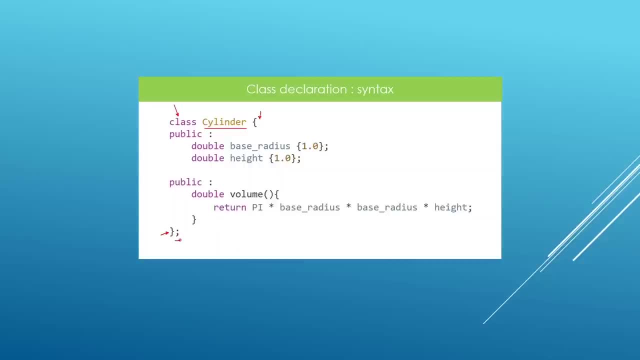 the properties that your class is going to have. In this case, we have two properties That really define a cylinder: We have the base radius and we have the height. We have decided to model these things as double types inside our class, And this is going to make the first part. 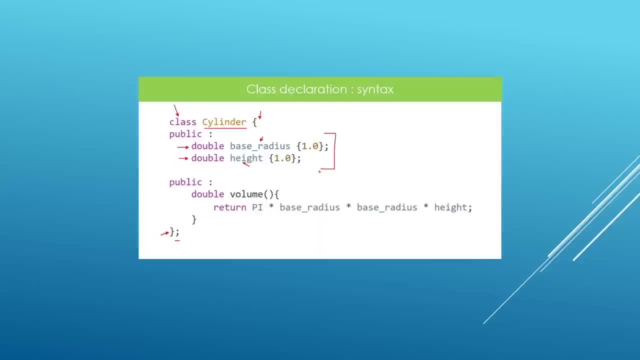 of our class, The member variables. The second part is going to be made of behaviors or functions that do things on the class using the properties, And one function we have is the volume function, which is going to help us with the number of variables, And this is going to help us with the 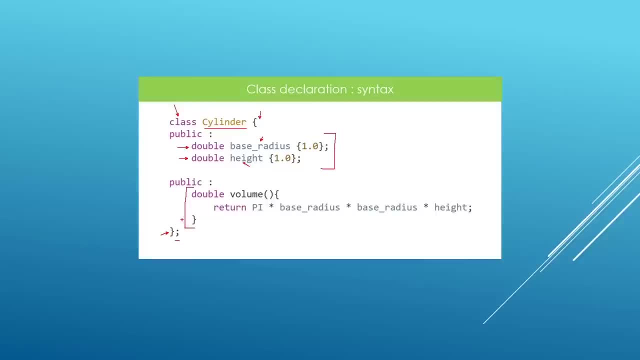 volume of our cylinder. here, If you look at its syntax, it really is a function. We have a return type, We have the name of the function, We have the parameter list, which is empty by now, And we have our curly braces that delimit the body of our function Inside the function we're going to do. 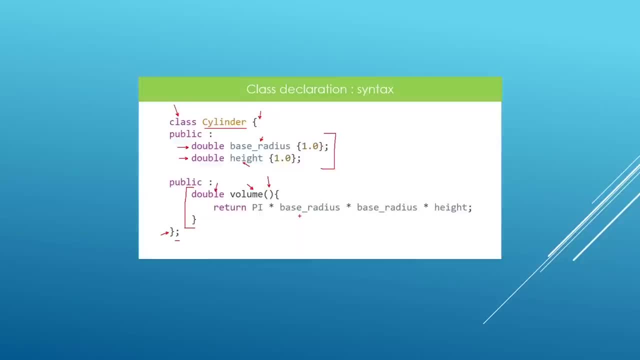 nothing special. We're just going to return the volume of our function here And, if you remember, the volume is the base area multiplied by the height. And if you remember, the volume is the height And this thing here is going to model the base area. You see, it's pi multiplied by the. 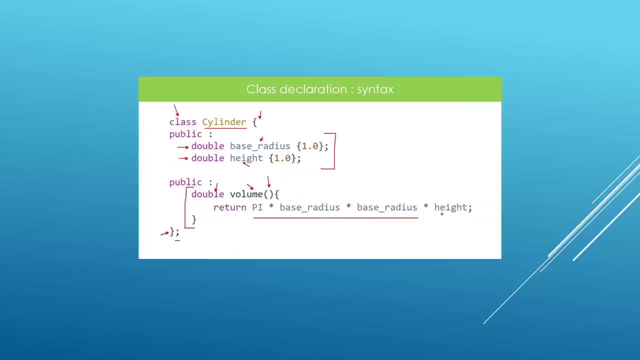 square of the radius, And then we're going to multiply this by the height And we're going to return the volume for use by whoever is calling this function. One thing we haven't really talked about is this public thing you see here, And what this says is that the members that we have in this 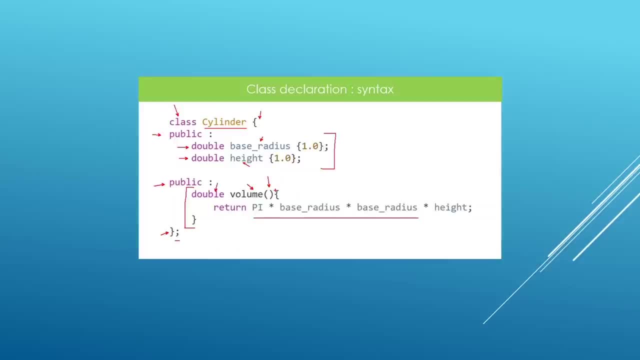 class are going to be accessible from the outside, So we're going to return the volume of our function outside of the class. For now we can't really understand this, But when we hit Visual Studio code, I'm going to show you what this exactly means. Now that we have the class declared, we can 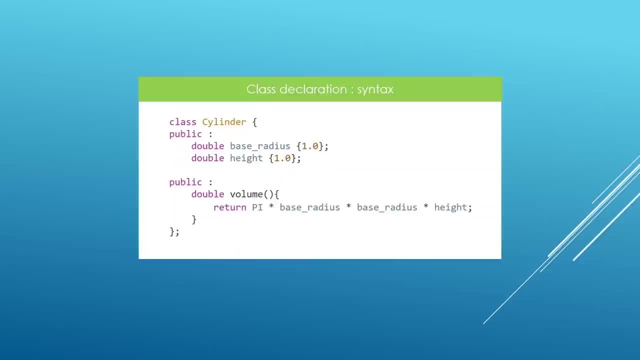 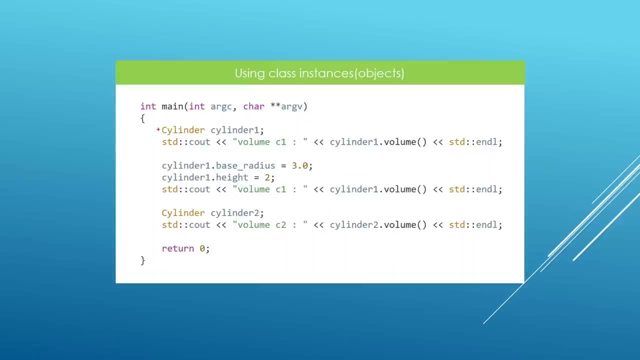 really use it like we use any other types. in C++, For example, we can head in our main function and set up a variable called cylinder one- as you see here, Its type is going to be cylinder- And notice that this is really a type that we build ourselves And we can really use it. 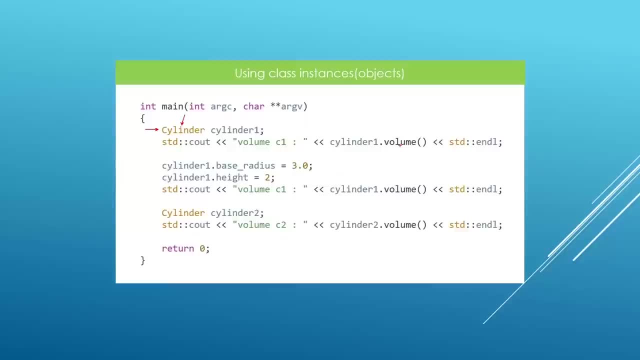 like we use other variables. For example, we can call its function using the syntax here and print the volume. This is going to print the volume using the volume function that we just set up in a minute. If we go down, we can modify things about our cylinder. For example, we can use the. 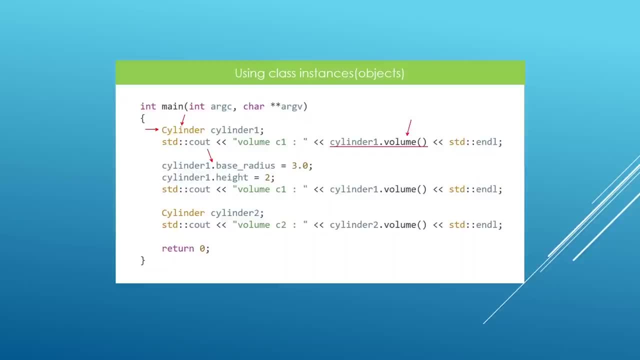 dot notation here to change the base radius and change the height. And if we try to print the volume again, this information is going to be picked up and be used by the volume function To compute the volume of our cylinder here. This is really cool. If you want, you can also set up. 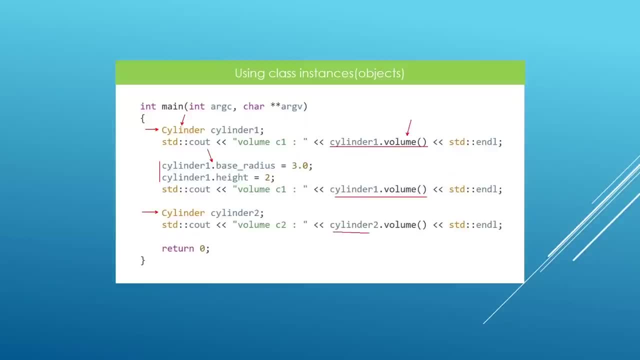 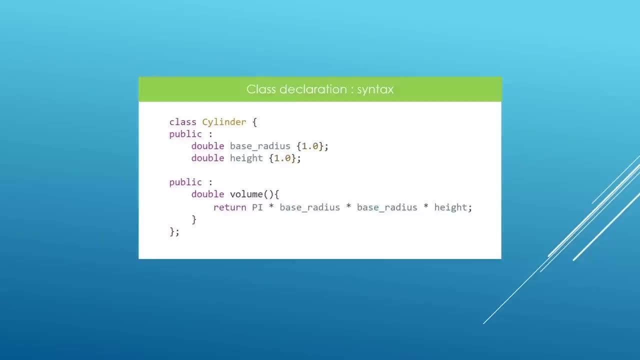 another cylinder like we do here, and we're going to print the volume And we can really do all kinds of crazy things with our types like this. Okay, this is our class and we can really use it to do a lot. Before we head over to Visual Studio code and play with us, I want to bring to your 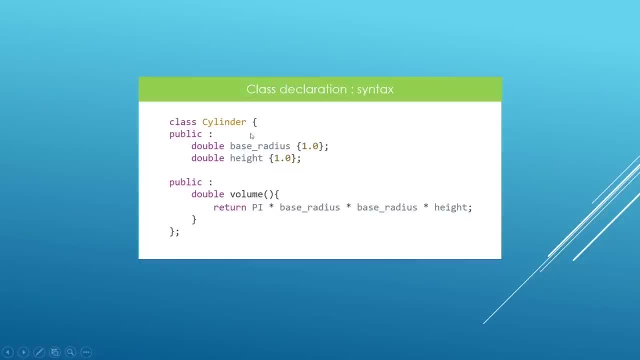 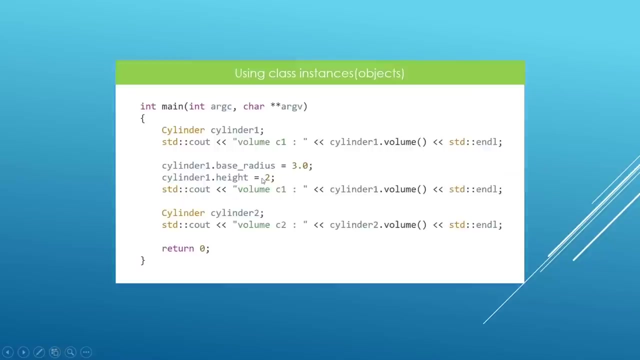 attention that members of a class are private by default, And what I mean by that is that they are private, And what I mean by that is that, for example, if we don't put this public keywords in here, we won't be able to use the volume function, for example, like we have used it in our main. 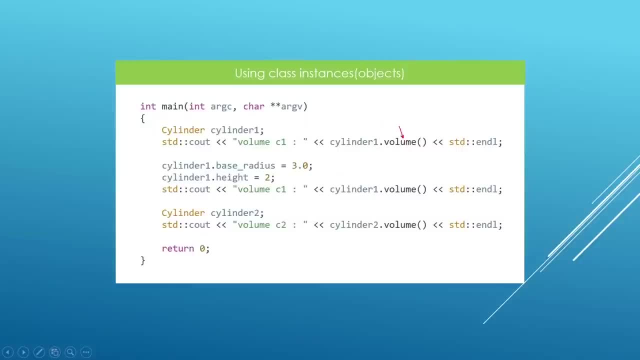 function. as you see here, If the member is private it won't be usable outside the class. This is what we mean here. We are trying to use this member in the main function outside the class definition. It won't be accessible if it is private. 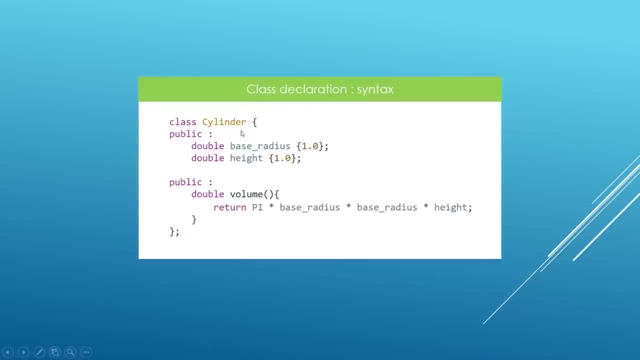 And we make it public by putting the public keyword and the column, like we do here. Everything after this public keyword is going to be public until we change this to private somewhere in our program, if we need that. Now that you have an idea about how you can declare and use your class in: 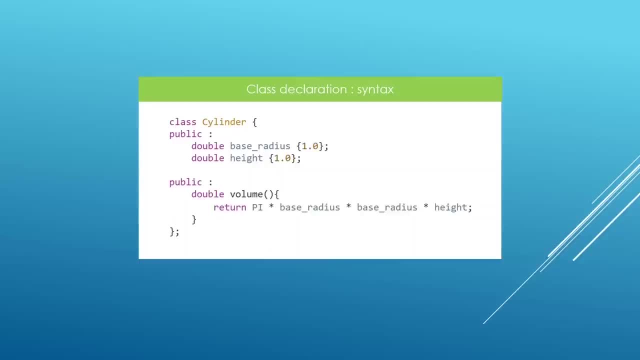 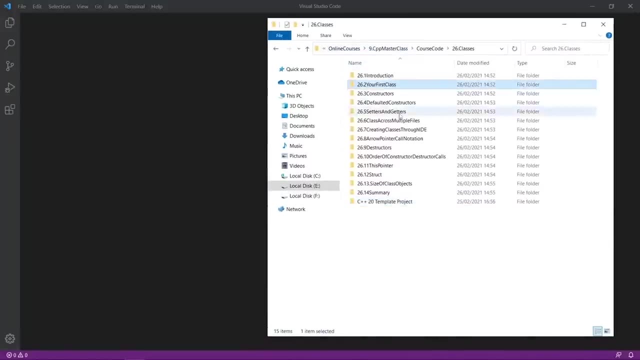 C++. let's head over to Visual Studio code and play with this a little more. Okay, here we are in our working folder. The current project is your first class. You are going to use it to do a lot of things. You are going to build your very first class in C++. We are going to grab our template files. 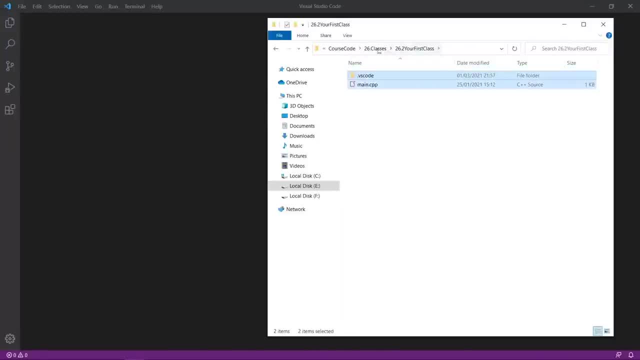 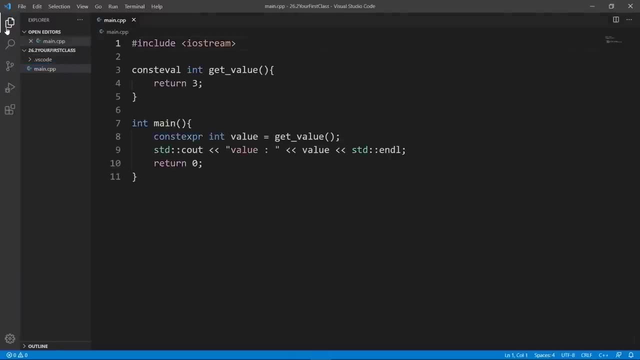 We are going to copy them and put them in place And then we are going to open this little guy in Visual Studio code by dragging and dropping here. This is going to open our folder. We are going to close the left pane here and clean things up a little bit. The first thing we want to do is to 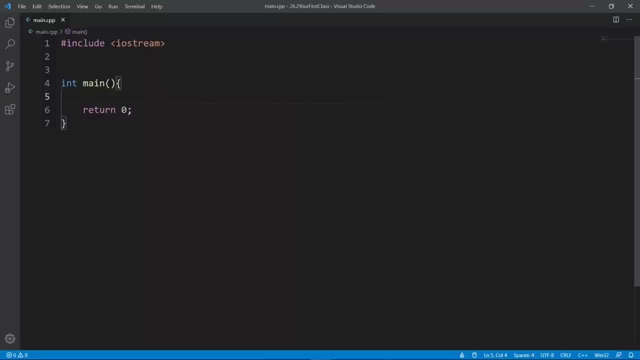 declare our class. But before we do that we are going to need the pi variable because, remember, we are going to model pi For use in computing the area and the volume of our cylinder that we want to model, like we did in the slides. So the way we're going to do that, I am going to declare a const variable and I am going 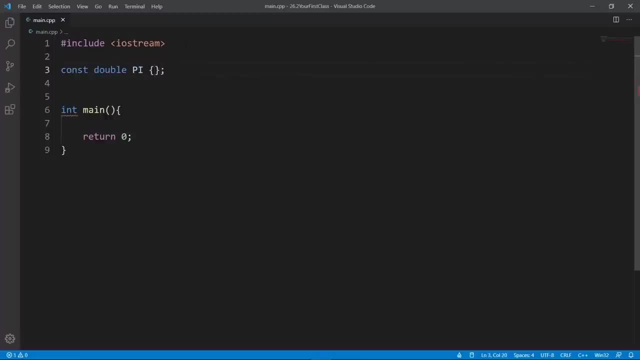 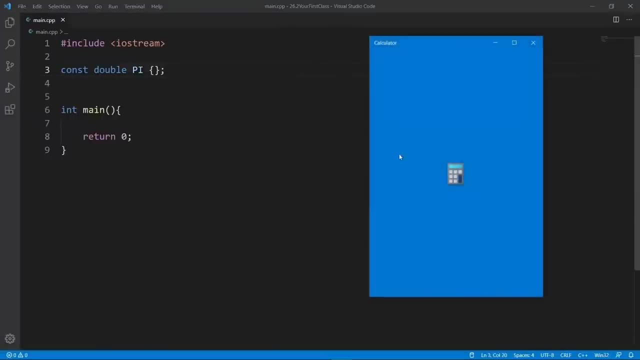 to call it pi and I am going to initialize this with pi To get pi. I'm going to cheat a little bit. I'm going to go in my calculator and let's see if I can get pi here and click on this, and I'm going to grab pi here and copy it. 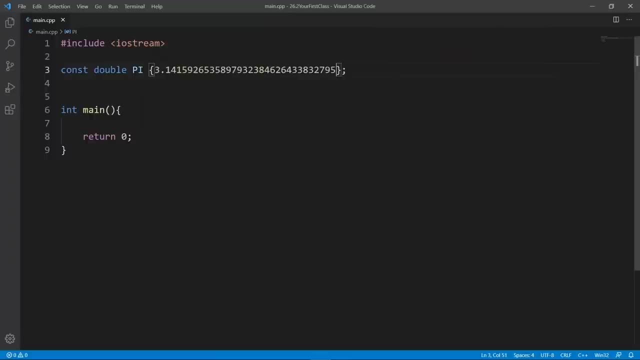 This is the easiest way I can find, So I'm going to put it in here and this is going to be our variable. Now that we have this, we're going to set up our class and to define a class, you say class, you have to put in this keyword, and then we're going to say the name of the class, The name of. 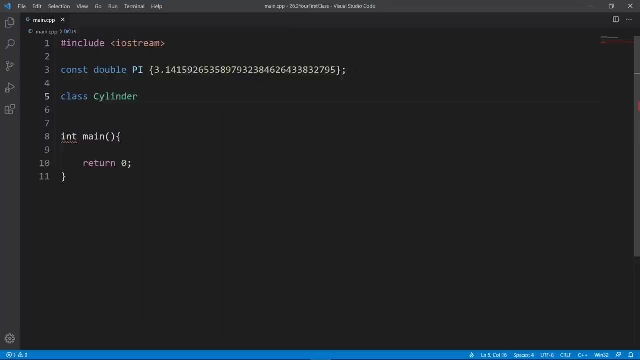 the class is going to be cylinder and after we do this we're going to put a pair of curly braces and we're going to end this with a semicolon. You have to remember this. if you don't put it here, the c++ compiler is going to complain. Now that we have the class blueprint here we're going to put in 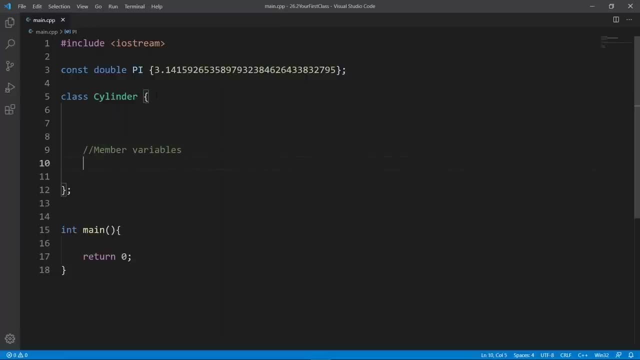 our member variable and these are going to be the variables we use to model the base radius and the height of our cylinder. We're going to put in a double variable and we're going to call this base radius and we're going to brace initialize this to zero. We can do this and we're going to set up. 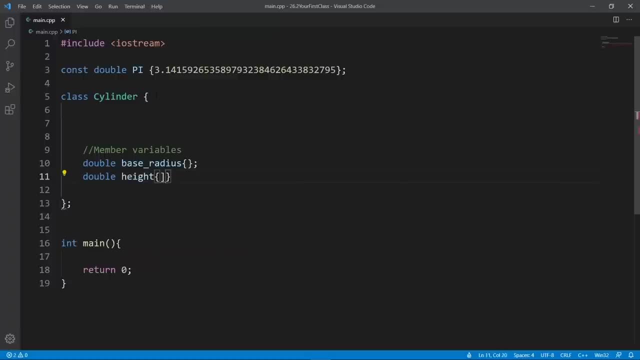 another one and call it height, and we're going to also initialize this to zero. Okay, now that we have this, we're going to put functions or methods in our class, and we do that by just putting the function definition in our class. so our function is going to be returning double because it's going 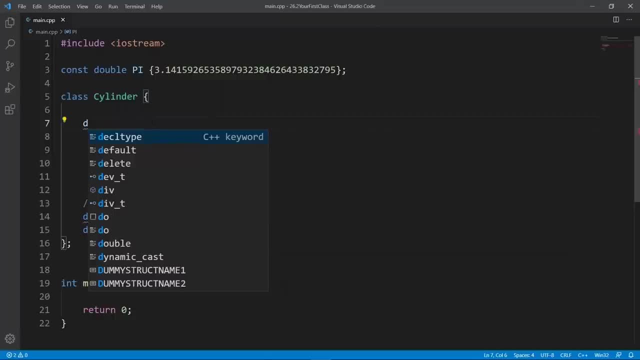 to be returning the volume of our cylinder. so it's going to return double. here the name is going to be volume and it's going to be computing the volume and returning that. remember the formula to compute the volume is going to be pi. we have our pi variable on top and we're going to multiply. 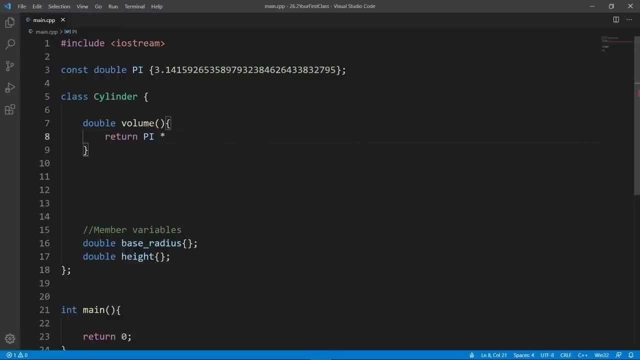 by base radius twice, because the base radius has to be squared. let's do that and multiply by base radius again, and then we're going to multiply by height and notice that these are guys declared in the body of the class. if i can say that this is the definition of the class we are able to use. 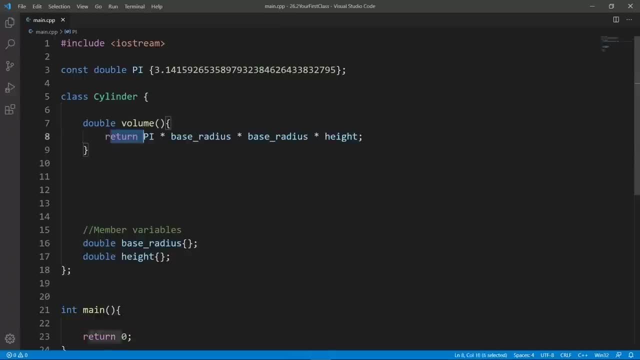 these guys because we are inside this class here. okay, now that we have this, our class is really defined, but we can't really use it quite yet. what do i mean by that? let's go in the main function and we're going to set up a variable of type cylinder. we can do. 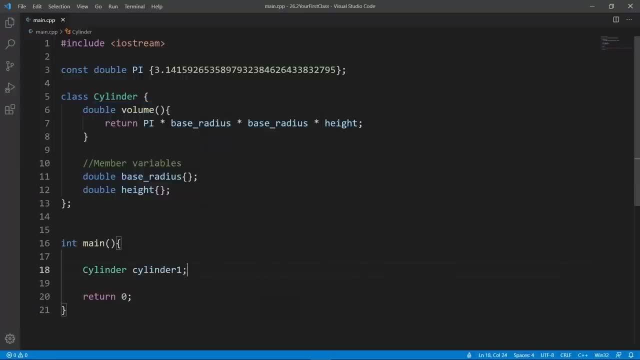 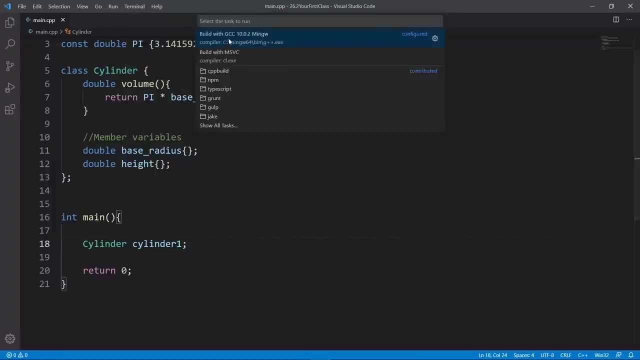 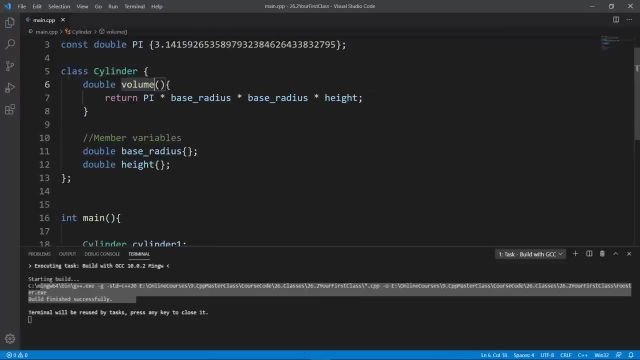 that, and let's call this cylinder one. if we do this and try to compile this, this is going to world. fine, let's do that. we're going to world with gcc world finished successfully. this is welding, but we have a function called volume here and we can try. 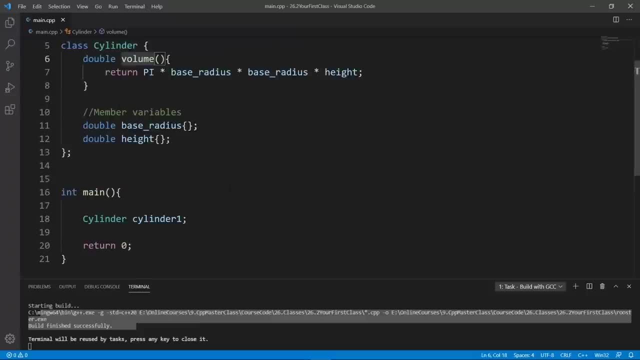 and call it using the dot notation that we saw in the slides. let's try and print the volume of our cylinder here and see what we get. so we're going to say volume- you can save that. and we're going to say cylinder one and do volume. okay, let's see if we can call this function here and the 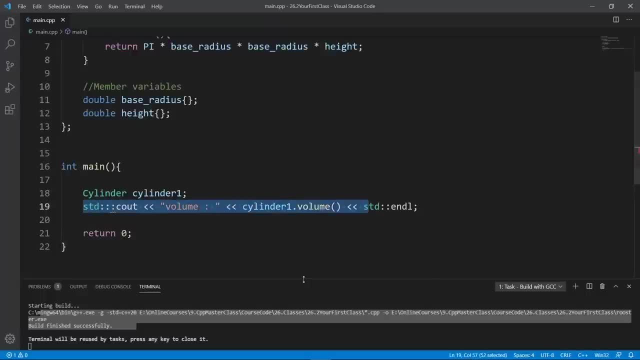 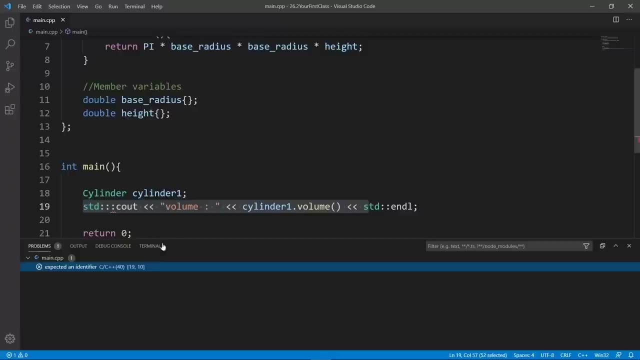 moment we do that, you see that we have a squiggly line here. so visual studio code has detected that something is wrong. let's hit the problems tab here and see what we get. it's going to say: expected an identifier on line. what this is not making sense. uh, we put three columns here. let's. 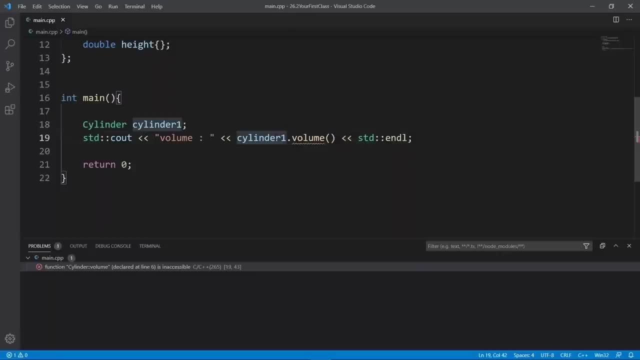 correct this a little bit and the error is going to change to be: cylinder volume declared at line six is inaccessible from this location here. this is what the error says, and it is inaccessible because members of a class are private by default. they want to be accessible from the outside of the class, like we are doing in the main function here. 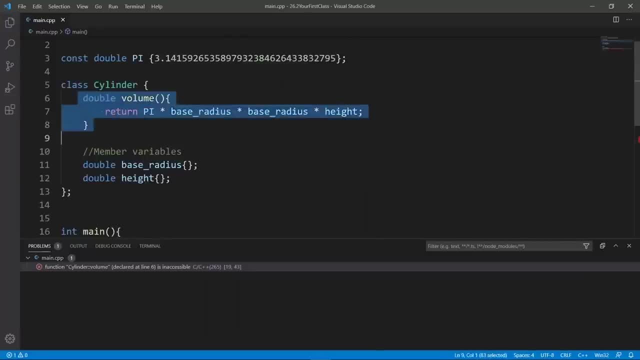 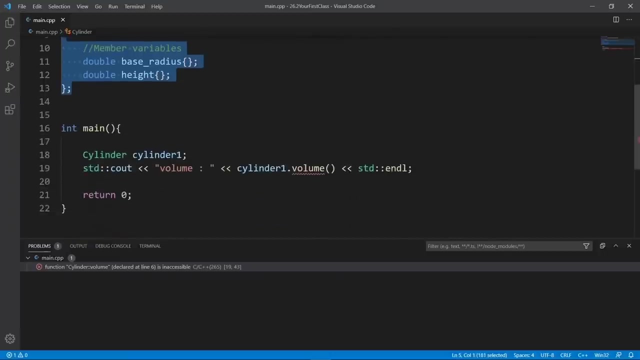 notice that we are able to access them from the inside of the class. you see, base radius is declared down here and we are able to use in the function because the function volume here is inside the class. so the members are accessible even if they are private. but private members can't be accessible. 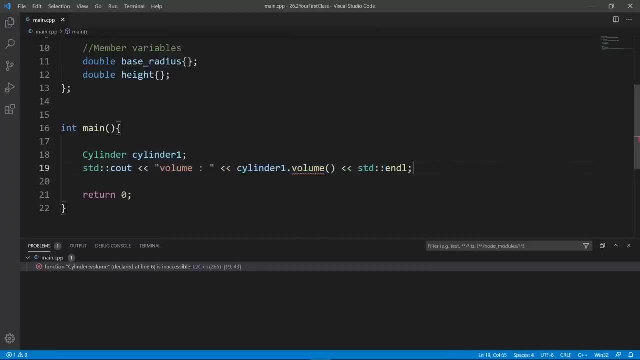 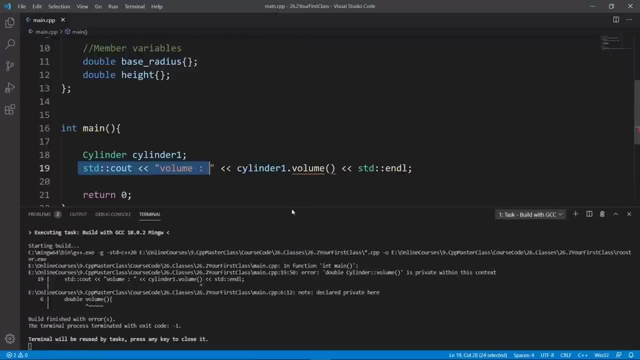 from the outside of the class, like we are doing in the main function here. that's why we have to this problem. let's see what the compiler says. we're going to pass this through gcc and we're going to get a compiler error. that we expect, and the compiler is really specific in this. it's going 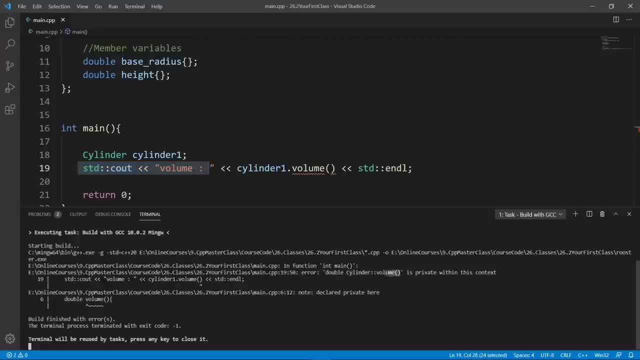 to say double cylinder volume. the volume function from the cylinder class is private within this context, and which context? the line 19 when we are trying to use it in the main function. so if you really want things inside the class to be accessible from the outside, you need to make 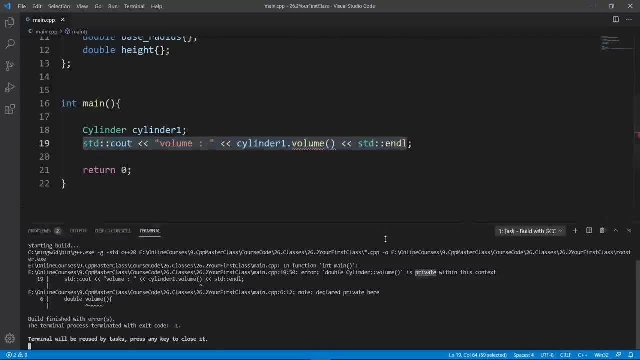 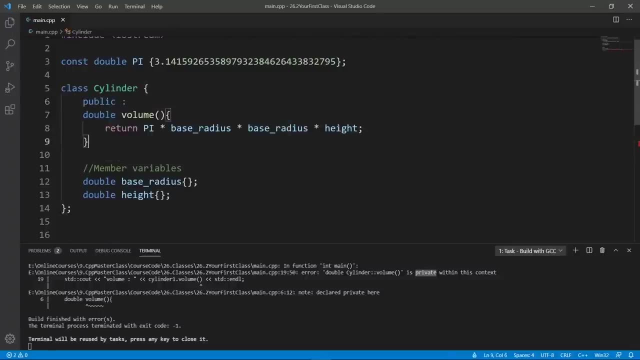 them public and change them from private. how do we do that? it is really simple. you use the syntax we saw in the slides. we're going to say public and put a column here, and when you do this, it is advised to align your things a little bit properly. so when we do this, everything after this public. 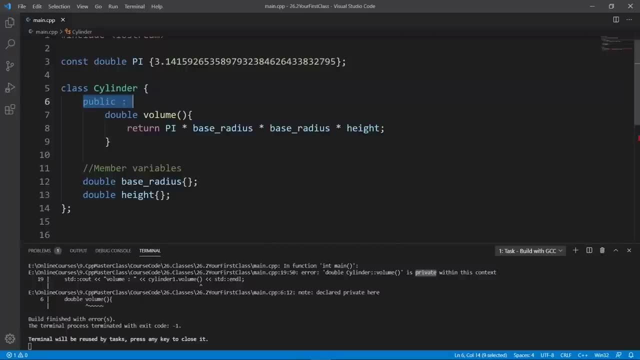 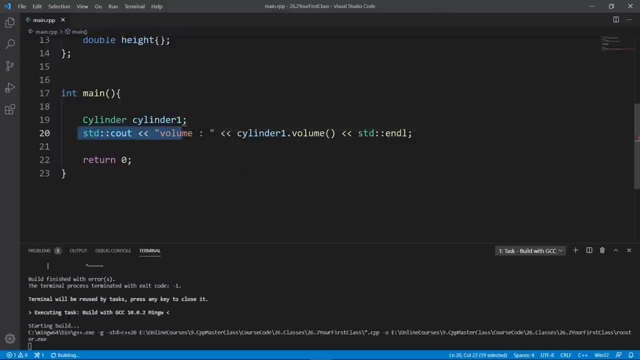 keyword is going to be public in this class and it will be accessible from the outside. let's try and build now, but before we build, let's show you that this quickly line should be gone. visual studio code is still confused. let's try and bolt, let's pass this. 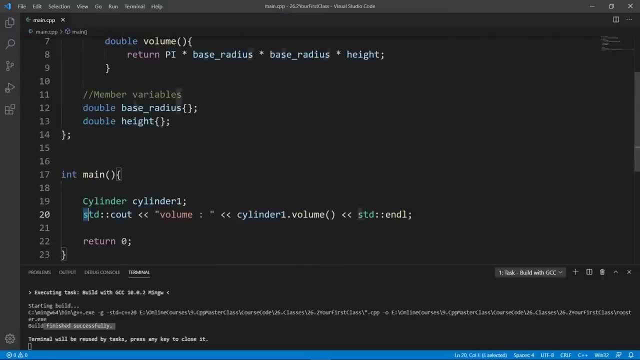 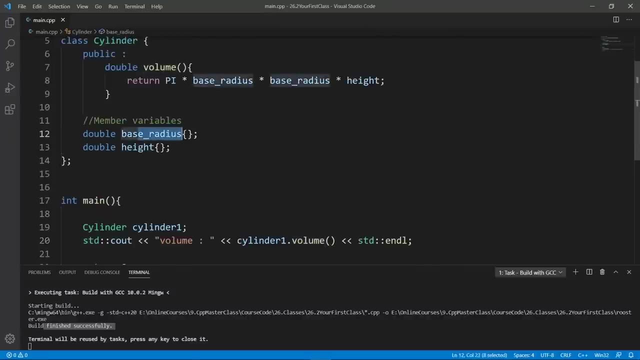 through gcc. now you see that the world is good. okay, now, if you try and print the volume here, we're going to get zero, because the base radius is braced, initialized to zero, the height is zero and if we multiply like this we're going to get a zero and return that. 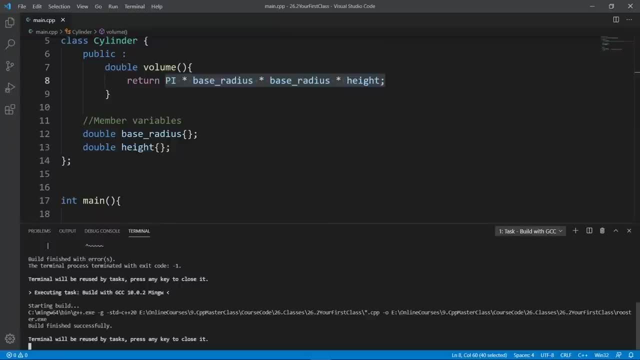 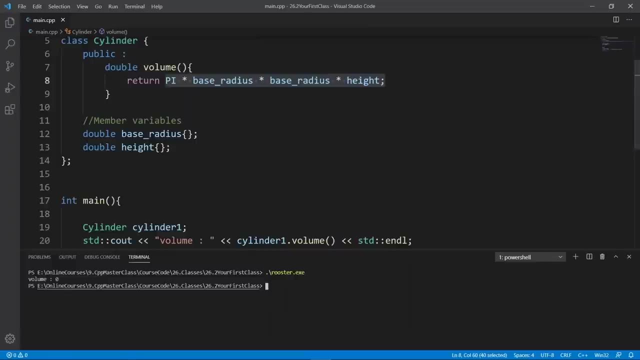 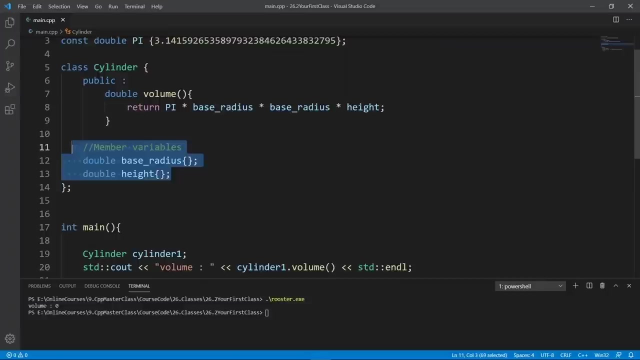 let's try and run this program, because we just build it successfully, we can bring up a terminal to do that, and let's clear and run rooster and we can see that the volume is zero and it is what we expect. okay, now our class is working, but there is really something bad about it, and that is: 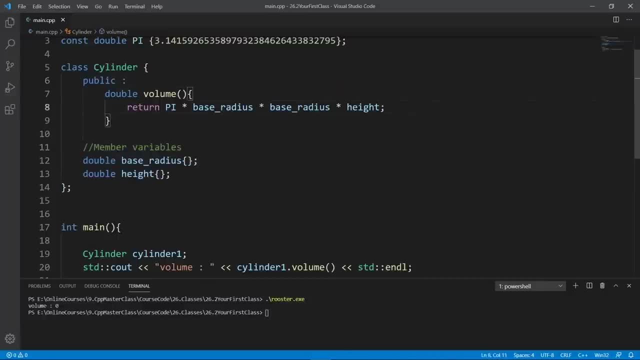 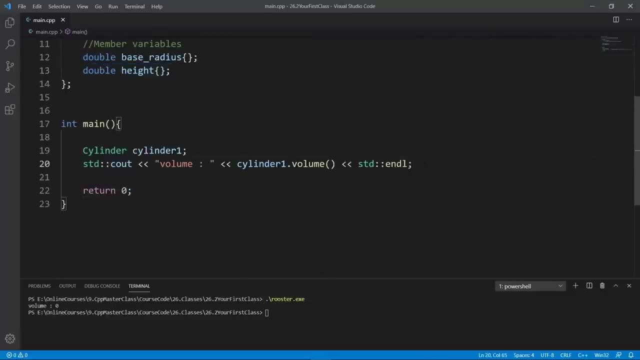 because the public keyword is going to make everything public in this class. the member variables are also going to be public, so we can go down here and print the base radius and the height, for example. let's do that and show you that this is the case. so we're going to say cylinder one and say base radius. this is going to print and we're going to 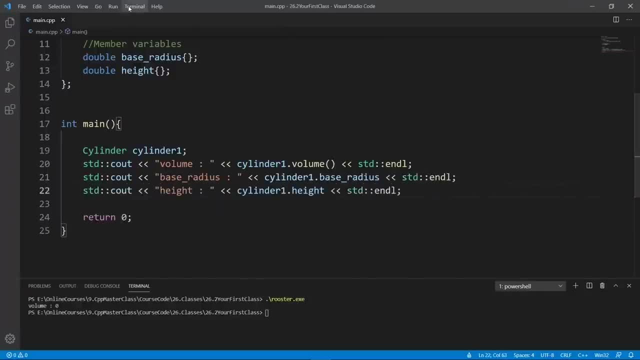 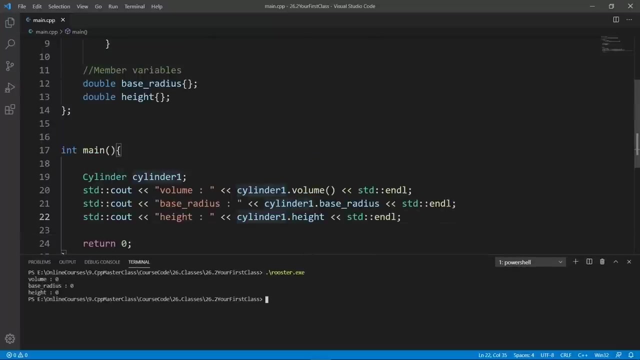 say height, we're going to print this out. if we try and print these guys, let's build and pass this through gcc. you see, the world is good and if we clear and run roaster, we're going to see that base radius and height are all accessible. to show you that this can also be different from: 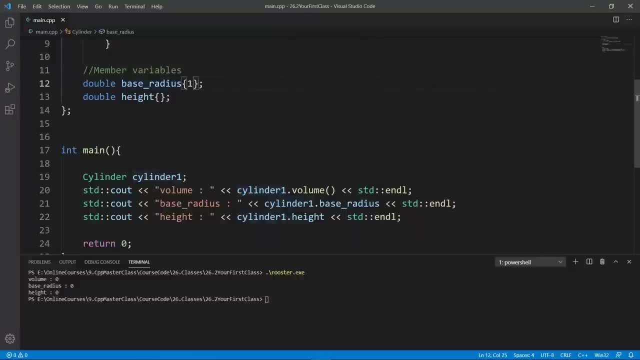 zero. let's change the base radius to one and the height to one to make it a unit cylinder. let's try and world. we're going to change these guys to one and the volume is going to be 3.14 or something. let's run rooster. we're going to see our volume here and we have the base radius and the height. 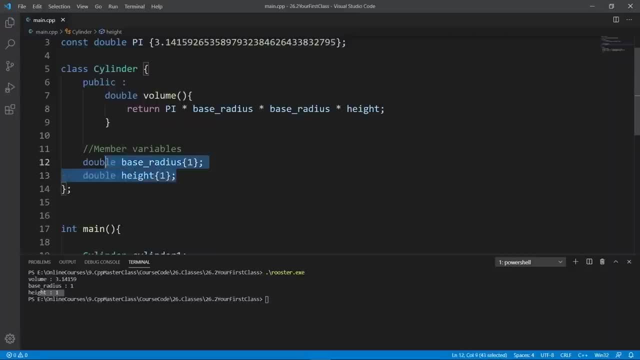 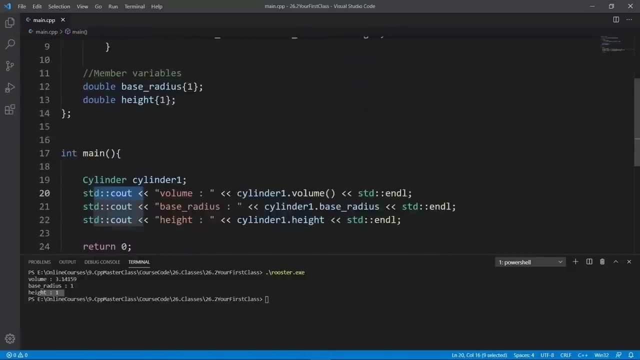 but this is really bad design because the member variables. in most cases you're going to want to keep them private from the outside. but if you want to keep them private, you can keep them private, because users of your class don't really care about the member variables, they just want to do. 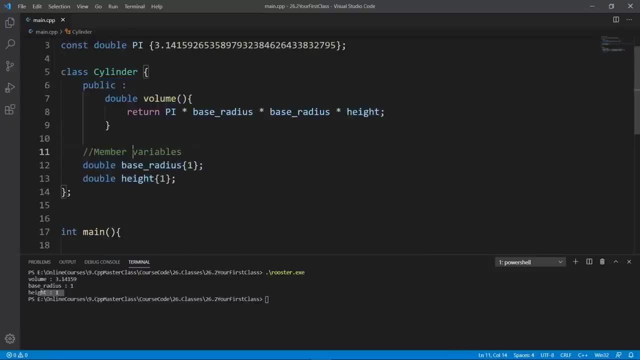 things with your class, for example calling the volume function here. so what we usually do in practice is to flag our member variables as private, and we can do that using the private keyword, as we do here, and at the moment we do this, everything after this private keyword is going to. 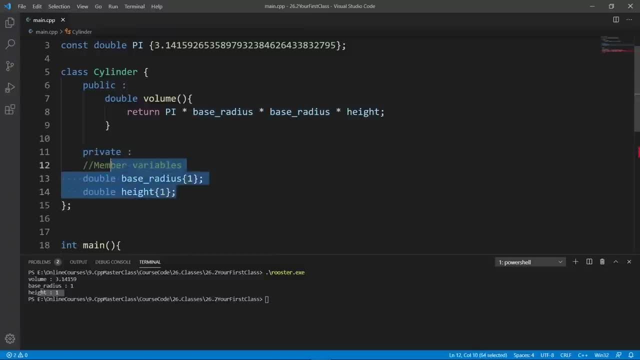 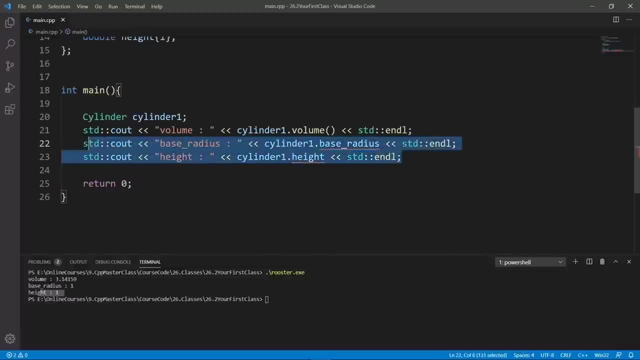 be private to the class. it is only going to be accessible from the inside of the class. but if we try to access that from the outside, we're going to get the same compiler error we saw before when we tried to access private stuff from the class in the main function here. 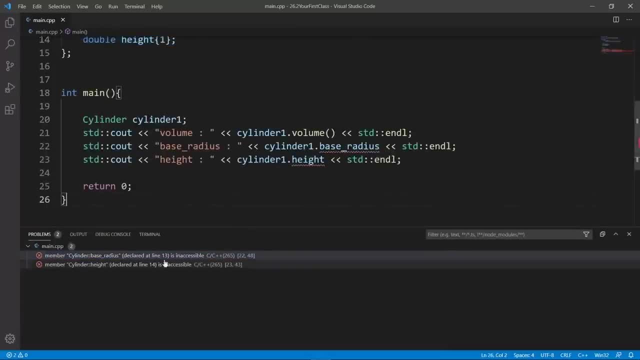 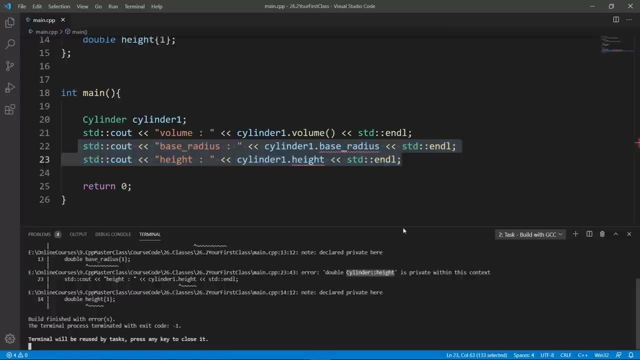 visual studio code is going to give us a problem saying that these member variables are not accessible from this context here, and if we pass this through gcc, we're going to get a clear compiler error saying that the height and the base radius are now private in the class and we can't access them from the outside. this is really what i wanted you to see. 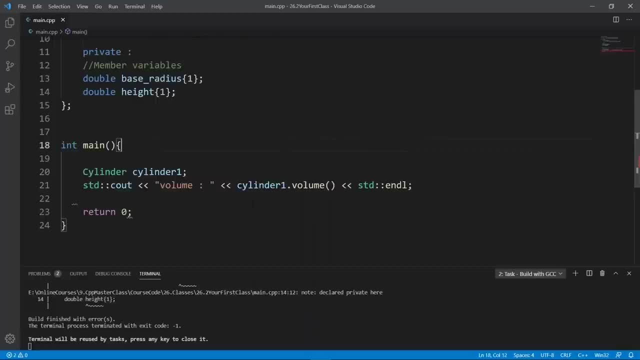 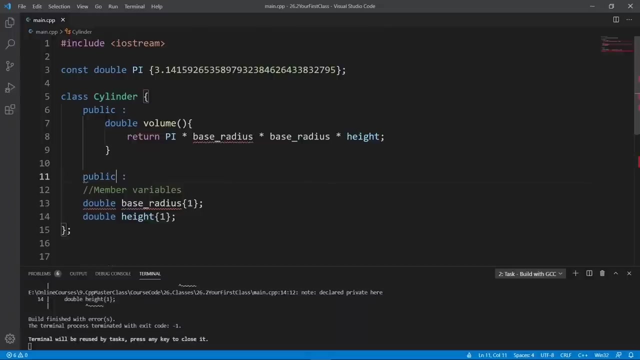 and this is good design. okay, now that we have our class declared and that we can use it in the main function, i want you to see that it is possible to change these member variables, but to do that we will need to turn this back to public, and we're going to see a better way to do this later. 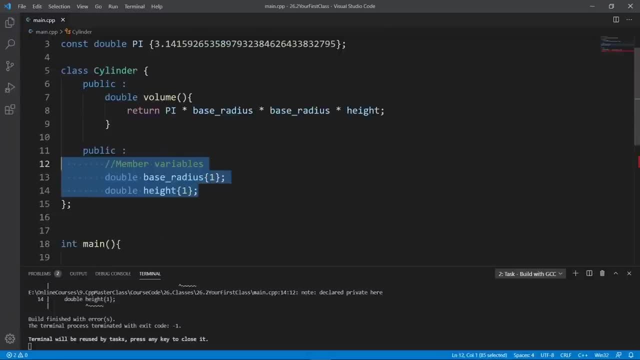 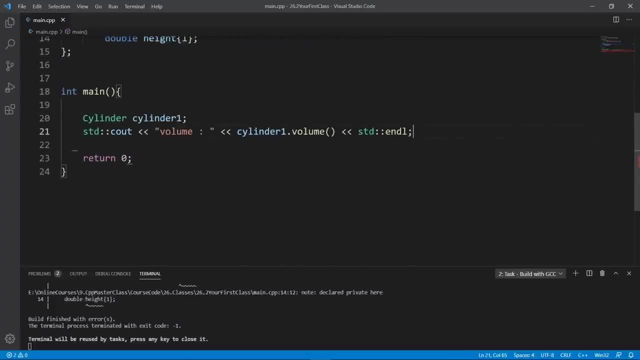 but for now, let's make them public and show you that we can change things around and make our members a little more interesting. so now that they are public, we can go in the main function and do crazy things: change the data. for example, we can change our member variables. 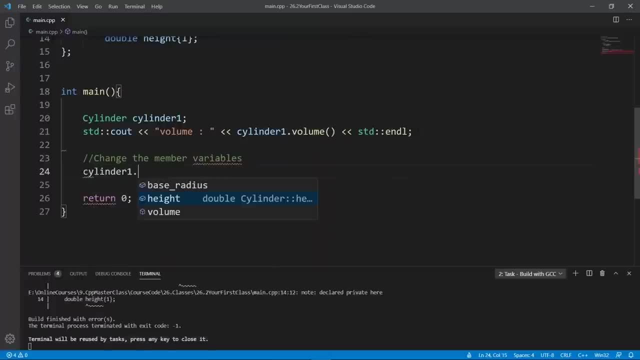 to be something else. let's go down and say cylinder one and say base radius. we can use the dot notation and put an equal sign and give another value to our base radius. let's make it 10, for example, and change the height to be something else. we can change that and we're going to put in. 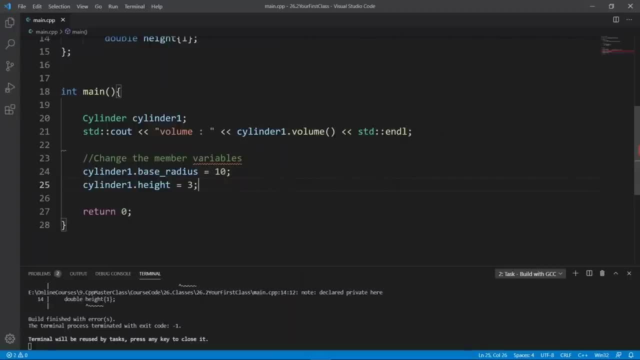 for example, why not now? if we print the volume again, we're going to get another value. let's copy this and put that down below our changes here. and if we build the program, it should build fine. the build is good, so we can hit enter and clear. and if we run rooster, we're going to get the volume to be. 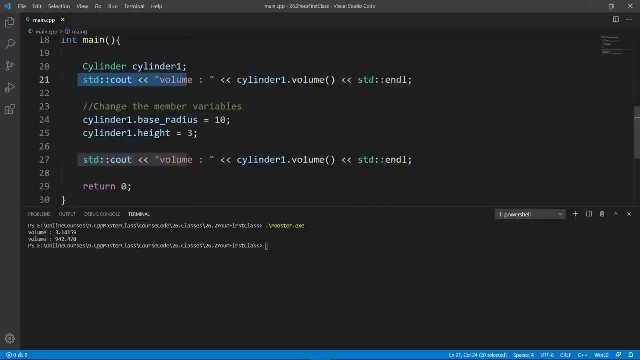 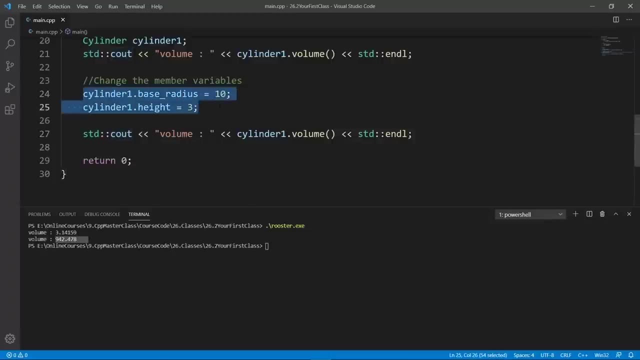 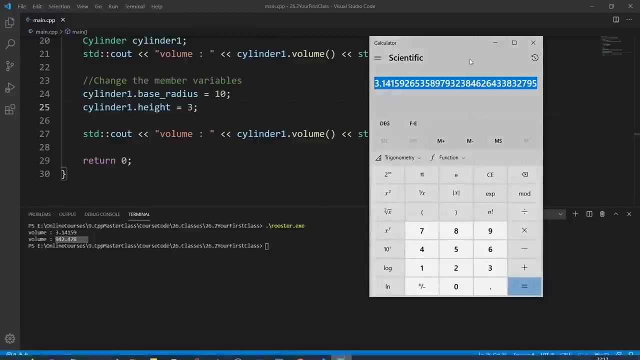 3.14. first here, the first line here and the second line is going to give us another volume and if we multiply these guys with pi and if we use our formula to compute the volume, we're going to basically get the same thing. let's try and prove this with our calculator. we have it around, so we. 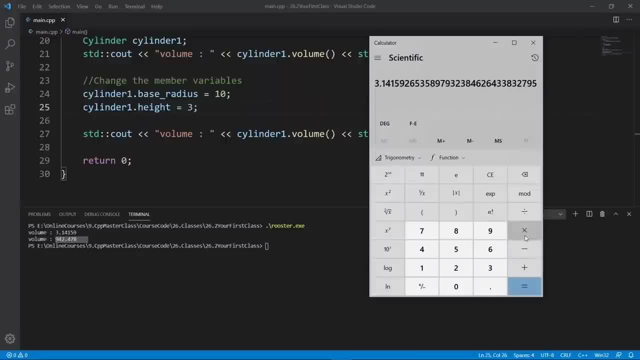 have pi in here. we're going to multiply this with 100, which is the radius squared. we're going to put 100 here and we're going to multiply this with 3, which is our height. let's put this in, and we have 942.47. 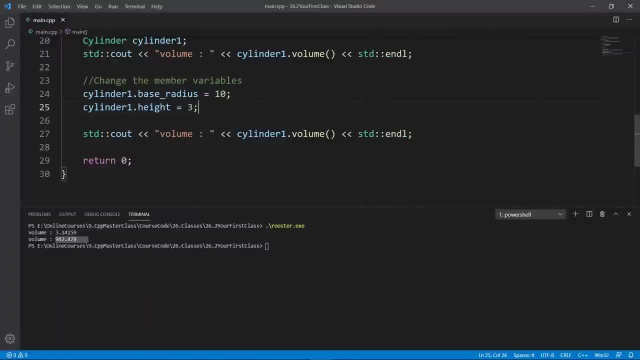 which is what we have here- roughly the same thing. so you see that our function is really computing our volume. we can even go down and change the height to something else. for example, we're going to change the height to let's make an eight and print the volume again. you can keep playing with. 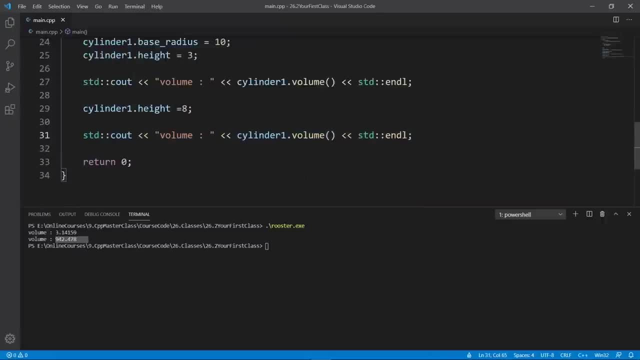 us and really make it clear that our volume function is computing our volume using the data that we have in the member variables. this is the message here: let's build again. the world should be. we're going to clear and run roaster. now we see another number for our volume and this is really 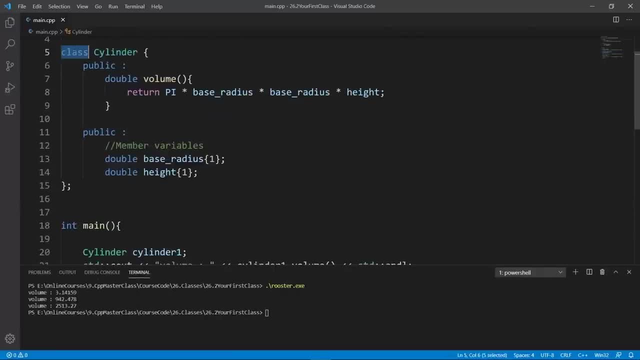 how you can declare a class again. you use the syntax. you see here: class, you say the class name, you put a pair of curly braces and you put your semicolon. don't forget this: members of your class are private by default, but you can make them public if you want, using 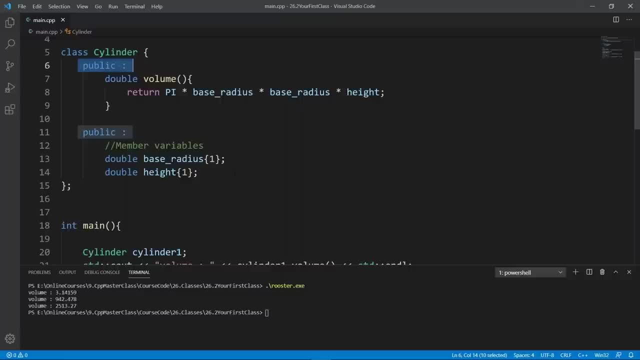 the public keyword, as we did here. inside your class, you're going to have two parts. you're going to have the member variables, which are going to be properties that define what your class is, and we're going to have functions or methods- let's say that- and these are going to be behaviors. 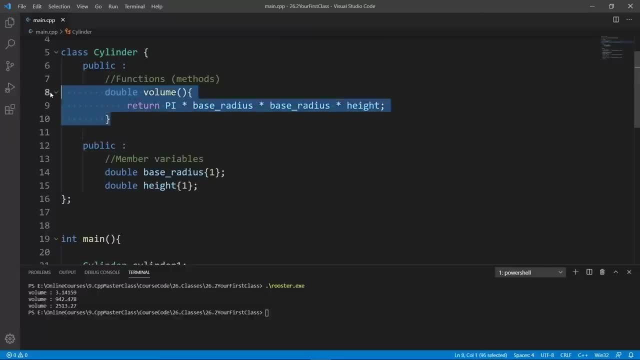 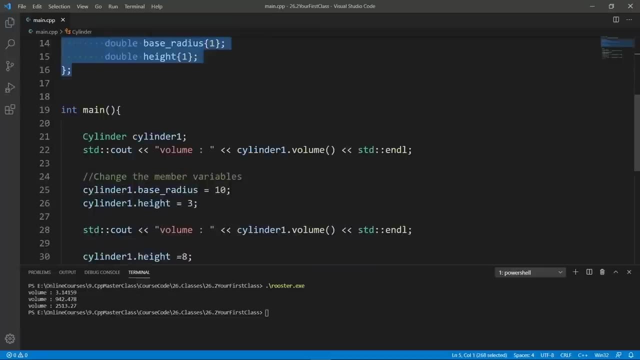 of your class you're going to go through. this functions to make your classes do things, and once you have the class definition in place, you can use it to create variables, as we do in the main function here, and the variables we create from our class are usually: 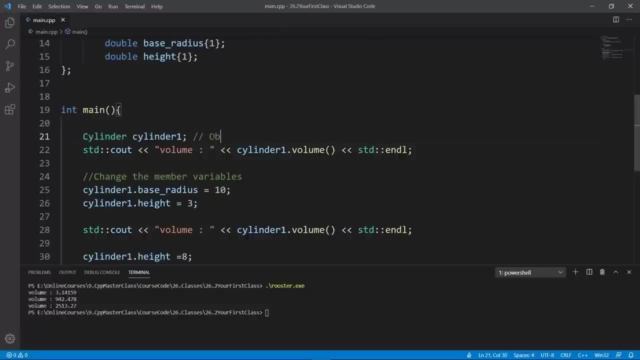 called numbers, which this work an a below. Sorry, we're going to use a number function and this's our class. we biz can령 and gradeed our own numbers. we define objects in c++ terminology- okay, the class is really a blueprint- and we create objects using. 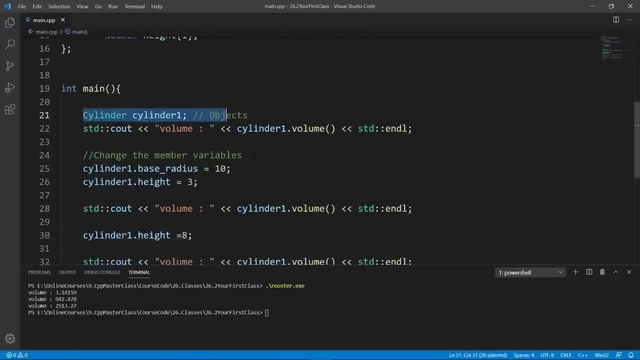 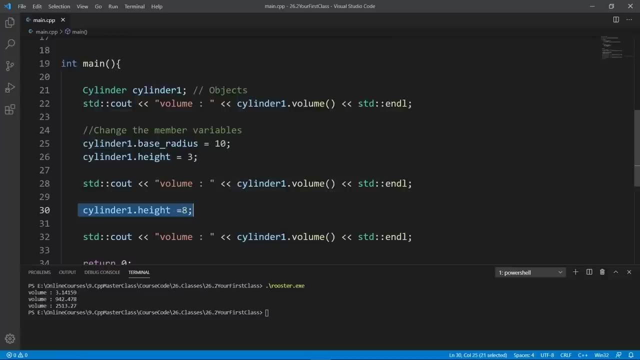 that blueprint and objects are going to have runtime data that we store in our class. okay, so, for example, if we hit this point here, the base radius is going to be 10 and the height is going to be 8 and that's going to be runtime information for our class object stored in this variable that 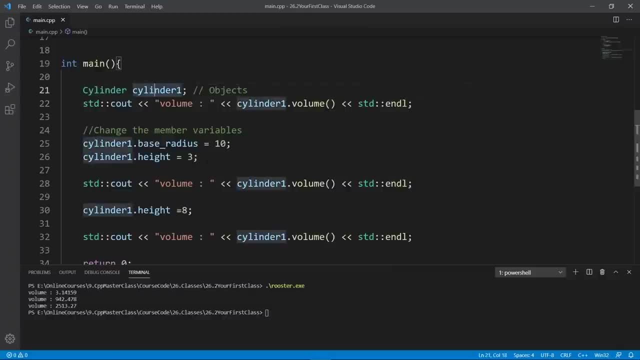 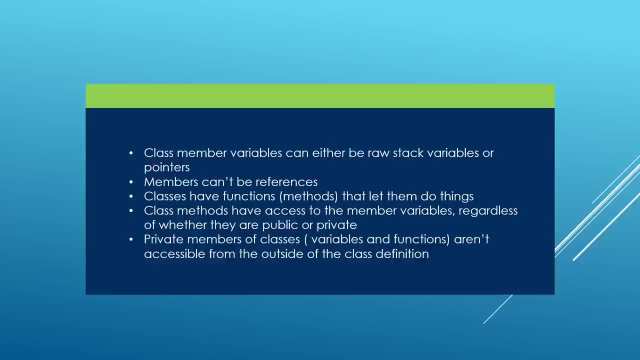 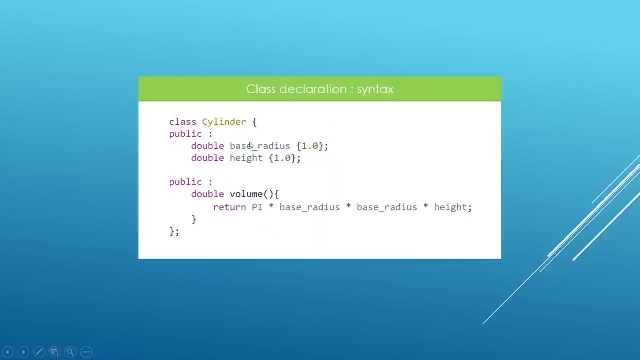 we call xylinder one here. this is really what i wanted you to see. okay, let's try and recap what we know about classes. so far, a class can have member variables, but so far we have used member variables as stack variables. if we go back, for example, you see that we say base radius. here you 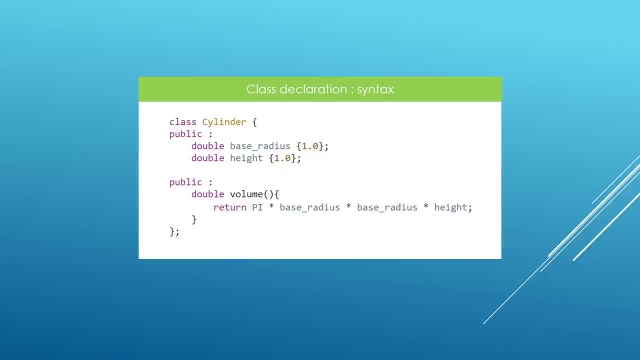 notice. it is not a pointer or a reference or anything. it is a stack variable inside our class. so member variables can only be stack variables, like we have in our class. so we have a stack variable inside our class, so we have a stack variable here. but they can also be pointers, but they can never be references, and the reason is a reference. 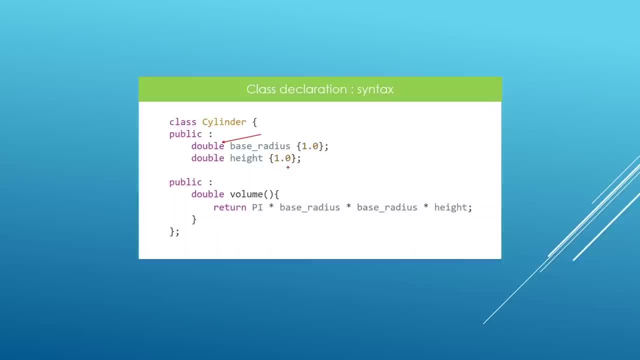 can never be left uninitialized and in the classes, when we declare member variables, the ability to leave them uninitialized is really important and we can't really do that with the references. i can't really go into the details of that, as we will see that as we progress in the chapter. 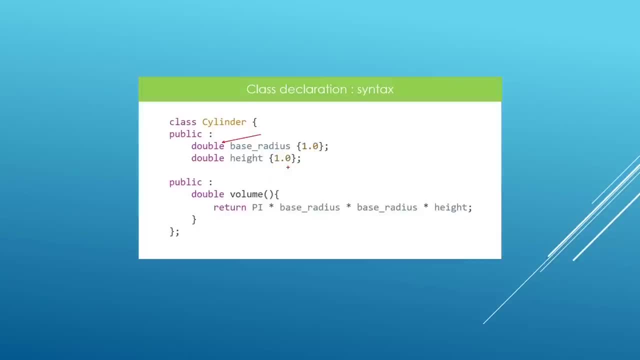 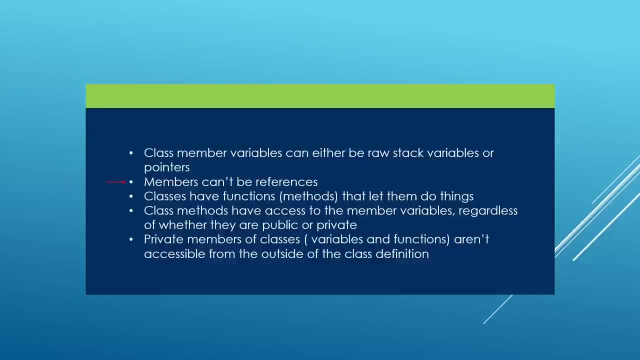 but note that member variables can either be stack variables or pointers, but they can never be references. in c plus plus- okay, that's what we just said here- members can't be references. classes can have functions or methods that let them do things. we saw an example of this with our volume function class methods have access. 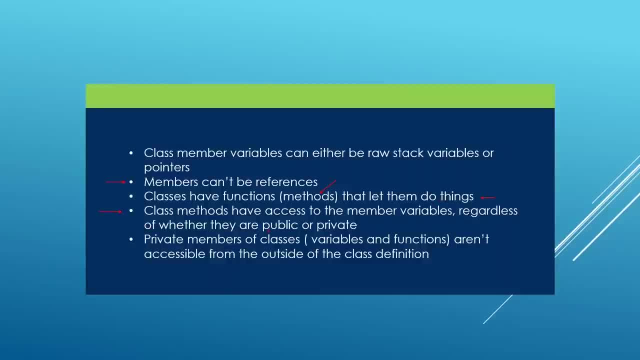 to the member variables, regardless of whether they are public or private. we have seen that the volume function will have access to our member variables, regardless of whether it is public or private. and, last but not least, private members of classes aren't accessible from the outside, as we saw in the main function. you can't access them. 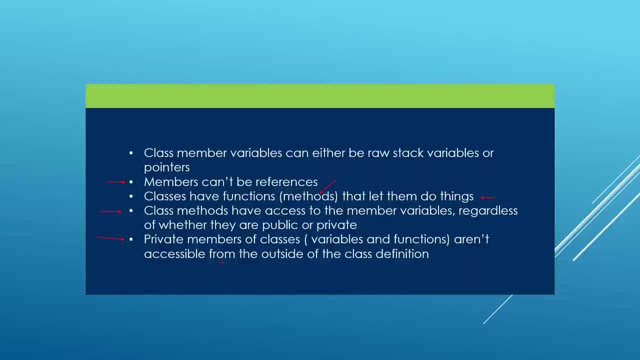 from the main function. you can only do that from the class definition itself. this is really all i had to share in this lecture. i hope you found it interesting. we are going to stop here in this one. in the next one we're going to see how class objects are built from construct. 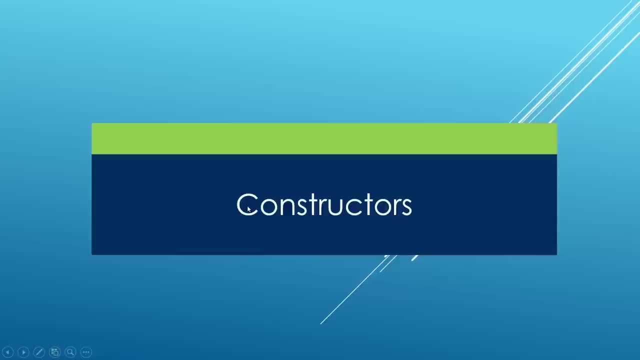 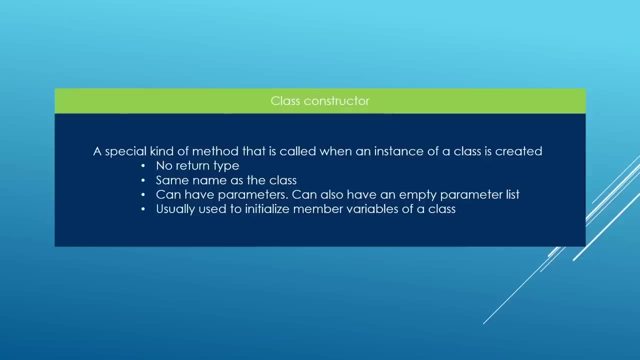 and constructors. go ahead and finish up here and make me there. in this lecture we're going to learn about constructors, and constructors are special class methods or functions that are called by the compiler to construct your class objects, and they are special because they have no return type. a constructor can never have a return type. as you see here, they have the same name as the class. 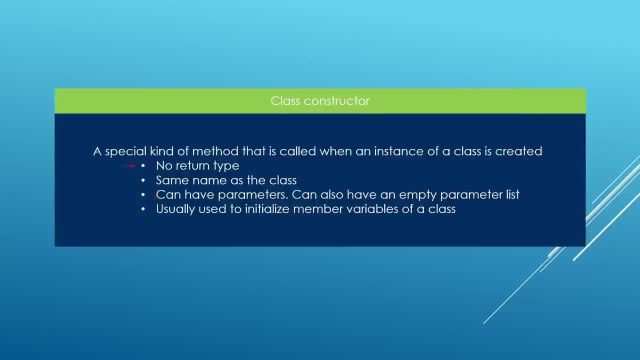 so, for example, our class in the last lecture that was called cylinder, the constructors are also going to have the same name as the class they are going to be called. also, cylinder constructors can have parameters, but if it makes sense for whatever it is you are trying to do, you can also leave the 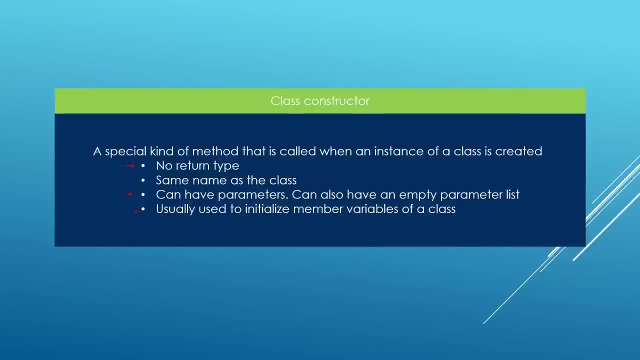 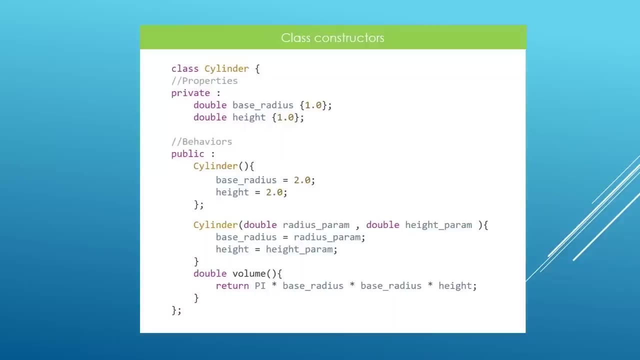 parameters out and constructors are usually used to initialize the member variables and put them in the state where you want them in your c plus plus application. let's look at how you can declare constructors for your classes. here is our cylinder class. you see, we have our member variables. we had 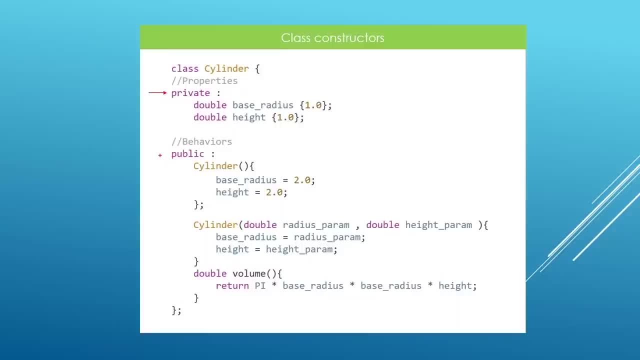 they are private now and we have a public section which is going to have our functions or behaviors. as you see, here the member variables are what we have seen from the last lecture, but if you look here, we have a few new things. here we have two things that look like functions but they don't have return values. that's something. 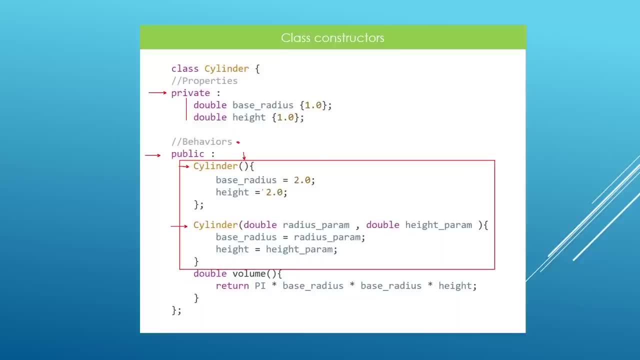 you should notice, they have a parameter list, as you see here, and we have a pair of curly braces, because these are really functions and these are special functions that are going to be called by the compiler to initialize your class objects. if you look here in this example, we are: 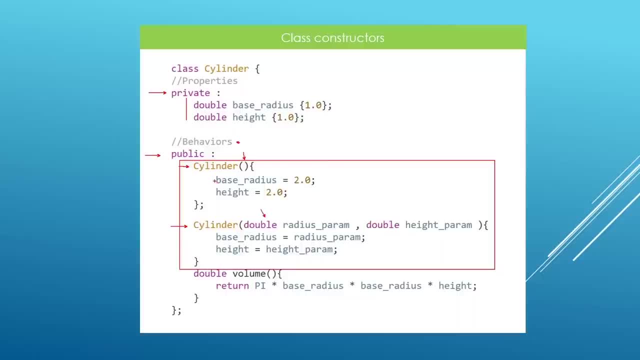 using the constructor with no parameters to initialize our member variables to two. and we have another constructor, as you see down here, which is going to take parameters directly and it's going to take the radius parameter and the height parameter. the parameters are of double type because that's what we expect in our class. 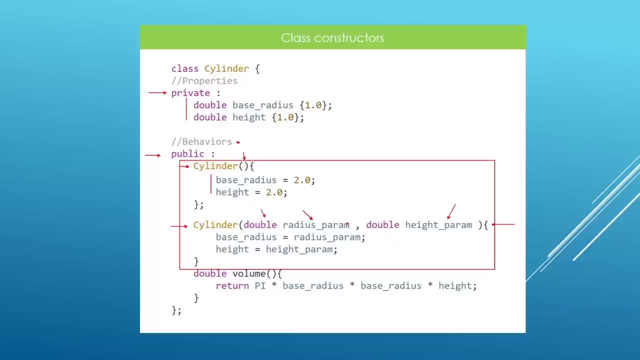 and we are passing them by value here because they are fundamental types and we don't really mind copying them. but please keep in mind that they are going to be passed by value and what you have inside your constructor body are going to be copies of the original arguments that were passed. 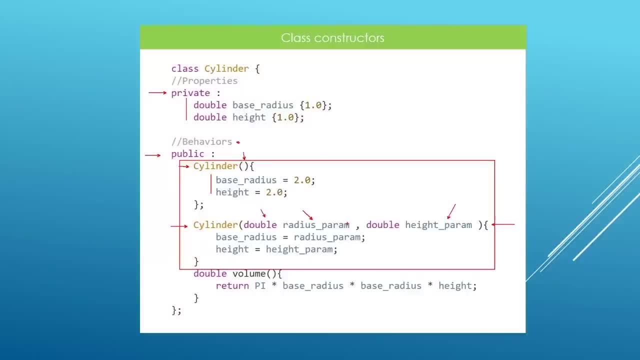 to your constructor, and this is really how you declare constructors for your c plus plus classes. constructors can either have parameters, like we have again on this example here, or they can have no parameters and this is going to be a default constructor. we're going to see that this is going to be called when you try to create variables of this cylinder type. 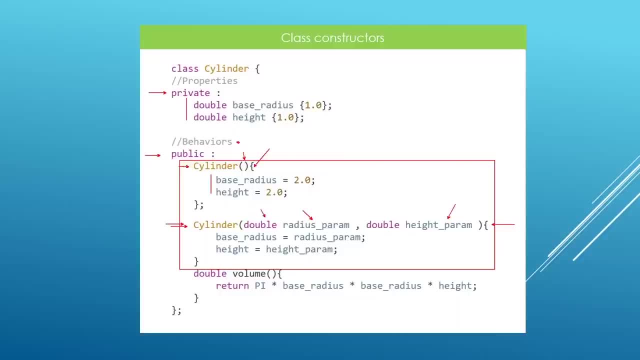 without passing the parenthesis like we do when we call this second constructor here. we're going to see this in a minute. okay, this is all i think i have to share in the slides about how you declare constructors. let's head over to visual studio code and play with this a little more, okay, here. 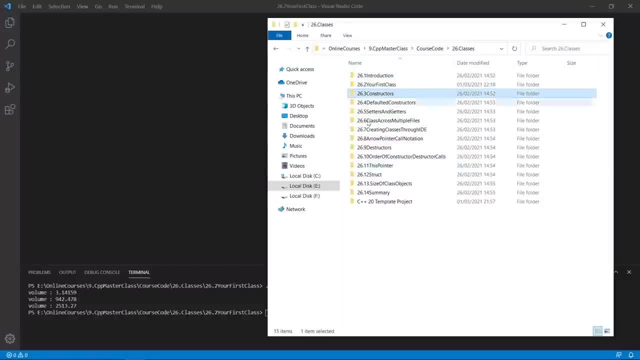 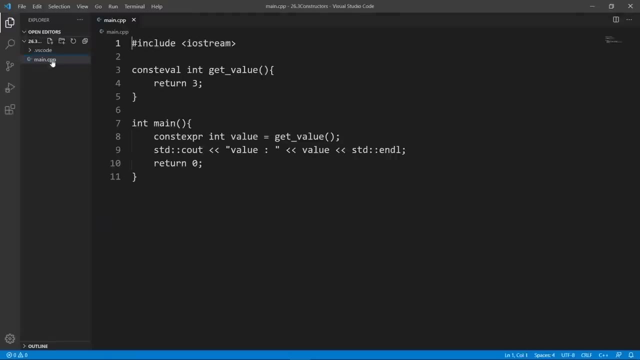 we are in our working folder. the current project is constructors. we're going to put in our template files pretty quick. let's do that, and we are going to open this in visual studio code by dragging and on top here this is going to open our folder. let's open our main cpp file and we're going to take 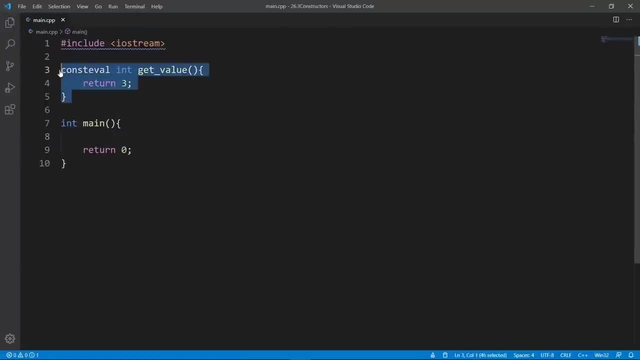 out what we don't need in the main function and on top here, and i am going to reuse code from the last lecture because we don't want to type that again. so let's put in our class definition. we have our variable pi, which is going to be used to compute the volume in the class here, and we 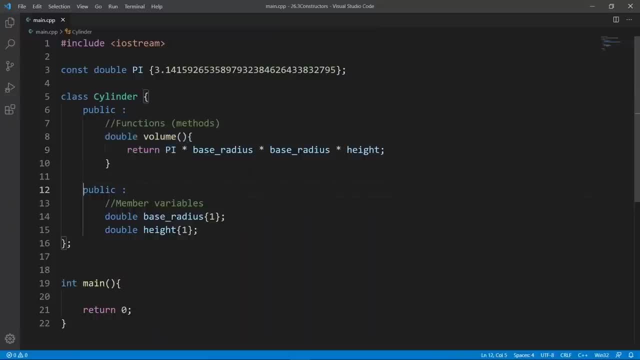 have member variables. okay, now that we are here, let's go ahead and create our class definition. let's change the member variables to be private, because making them public is really going to be bad design. it's going to expose them in the main function and people can mess with them. 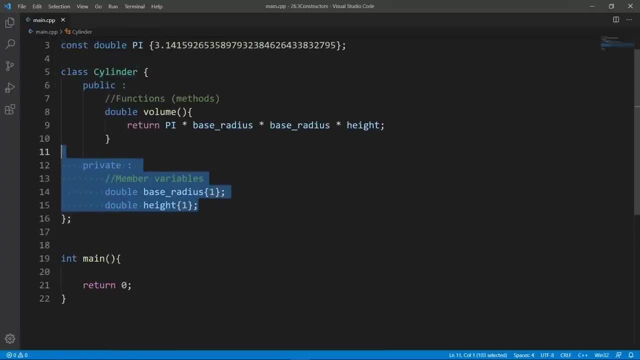 and really change the logic of how our class works. without our consent, it is advised to make your member variables private, unless you really have a compelling reasons to make them public. okay, now that we have our class here, let's set up constructors for it. so we're going to go down here in the public scope and say constructors, and we're going to set up. 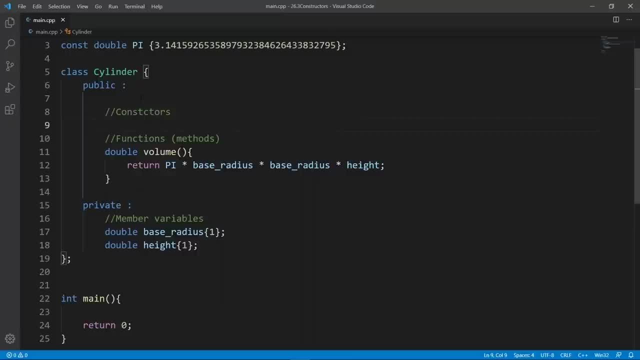 the first constructor, which is not going to take any parameter. so we're going to say the name of the class. remember, a constructor doesn't have a return type and it has to have the same name as the class. so we need to comply with that and we're going to put our pair of curly braces and 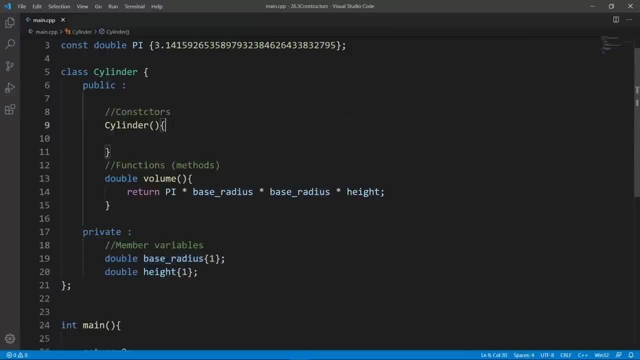 inside. we're going to initialize our member variables however we want. so what we're going to do here, we're going to set the base radius to something- let's make it a 2, like we saw in the slides, no problem with that- and we're going to set the height to something else. and we are going to set the height to 2 as. 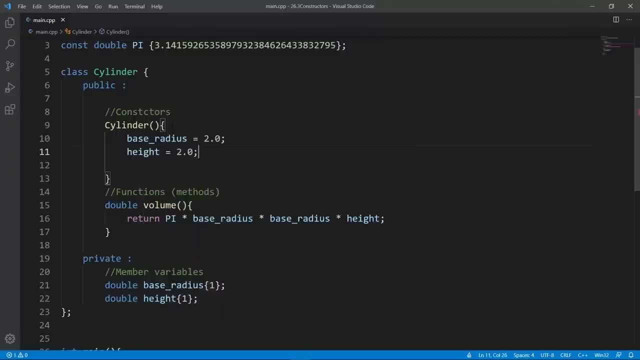 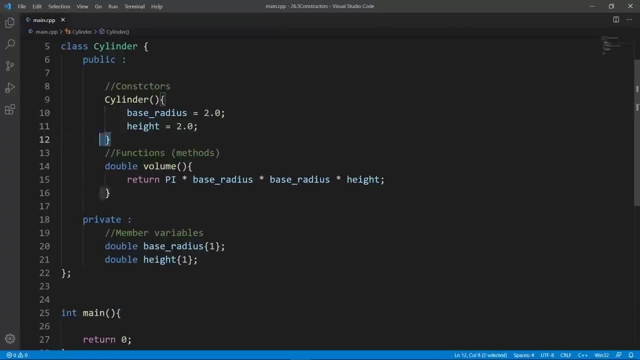 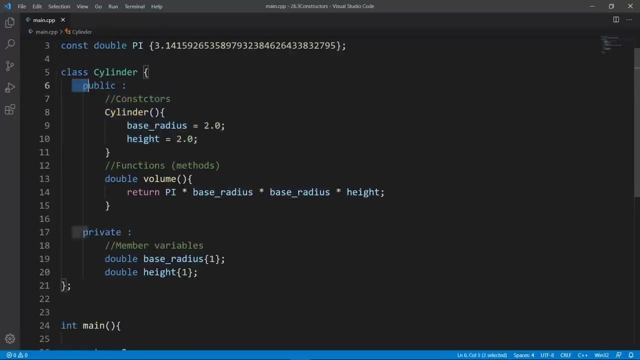 well, we can do that. you can use what you want, and now we have our constructor and it is initializing our thanks. okay, now that we have the constructor in place, how is it really called by the compiler and notice that our constructor is in the public scope of the class. if it isn't public, you won't be able to access it from the outside. 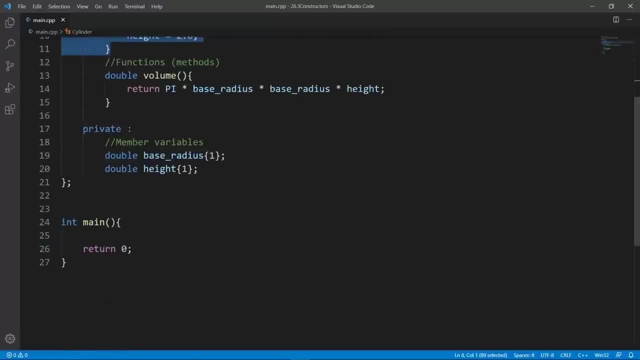 and the compiler will fail to build your objects and we're going to save this in a minute. but before we do that, let's try and create a cylinder object now. so we're going to say cylinder and say cylinder one, like we did in the last lecture. and when we do this, 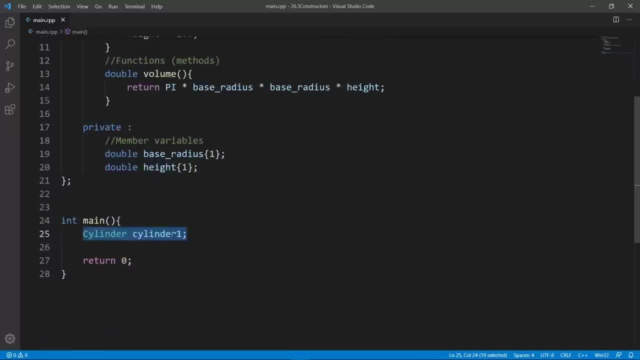 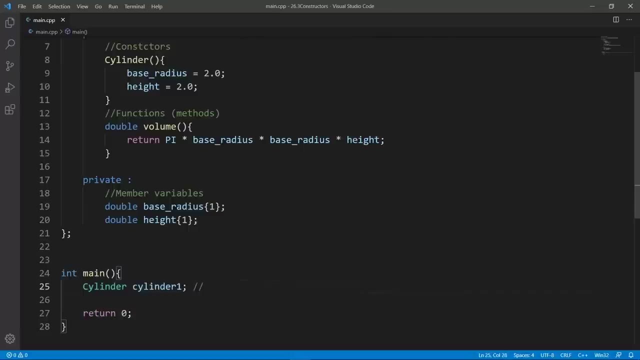 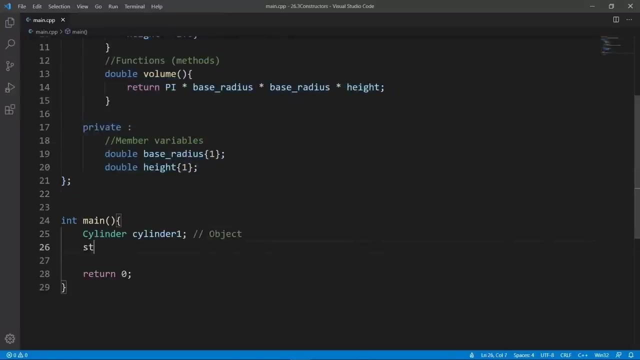 notice what we see if we print the volume of our cylinder object. here this is an object because we're creating this from our blueprint, which is the class definition here. you really need to know this. this is a class object, let's say that, and we're going to print its volume. we're going to 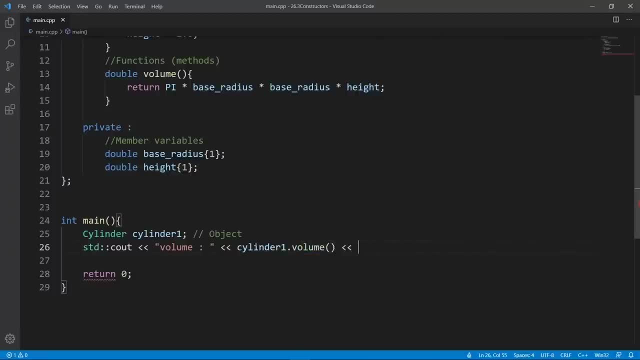 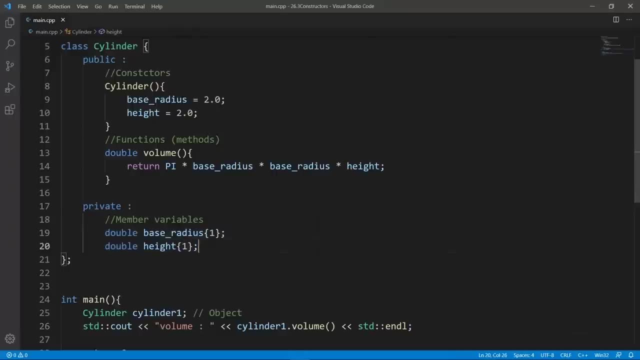 say cylinder one and we're going to call our volume method. we should say: and if we build, you're going to see that this is going to work, but the volume is not going to be coming from the initial values we have here, we will have changed these guys to two from our constructor here. 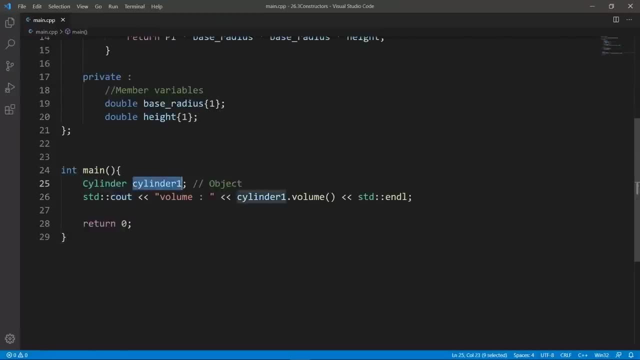 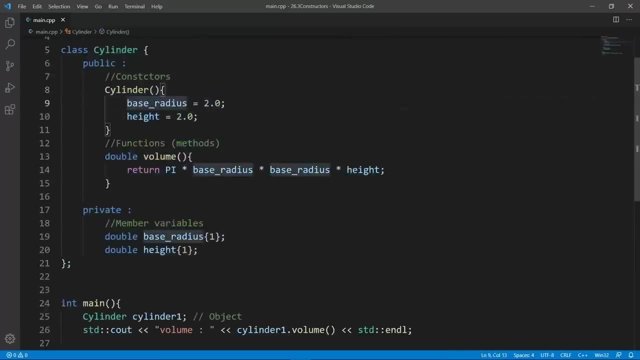 because the compiler is going to look at this line here and see that we are trying to build a cylinder object. it's going to look at the class definition and it is going to say: do i have any constructor that i can use to build an object from the syntax i see here? and it's going to see: 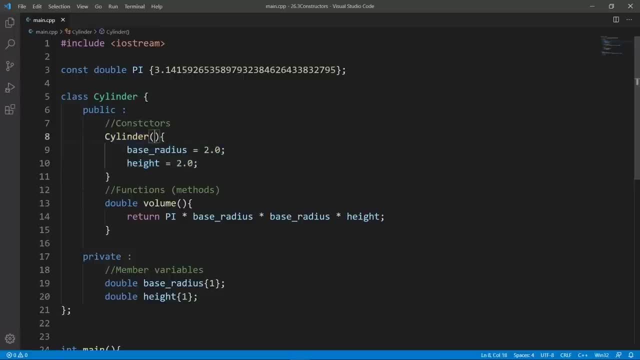 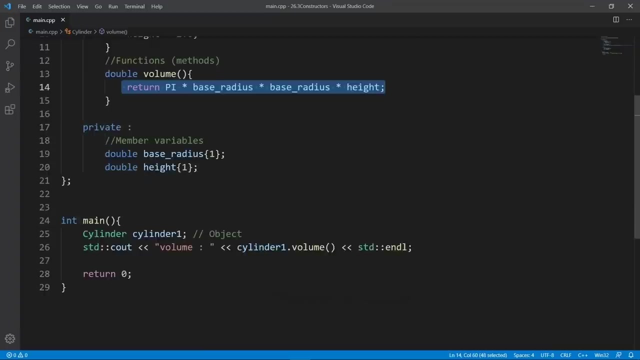 that it has a constructor that doesn't take any parameter and it's going to use it to build our object and it's going to be using this information to build our cylinder object. so the baser radius two, the height is going to be two and it's going to use that to compute the volume that we print. 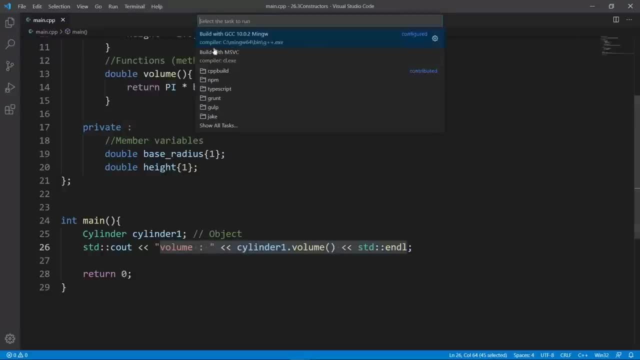 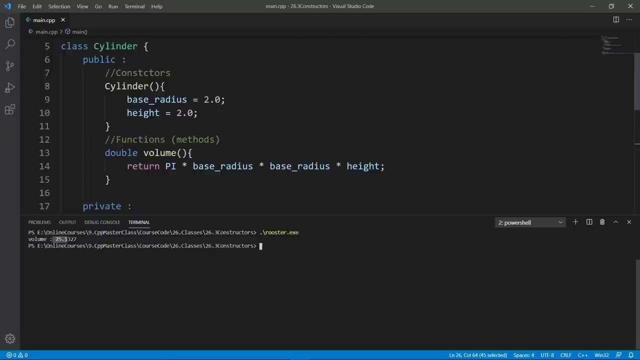 here. you really need to understand this. let's build and see if gcc accepts this. you see, the build is good. now we can bring up a terminal and clear and run rooster. you're going to see that we have 25, something which is a result of using this information we have here. if we take pi multiply. 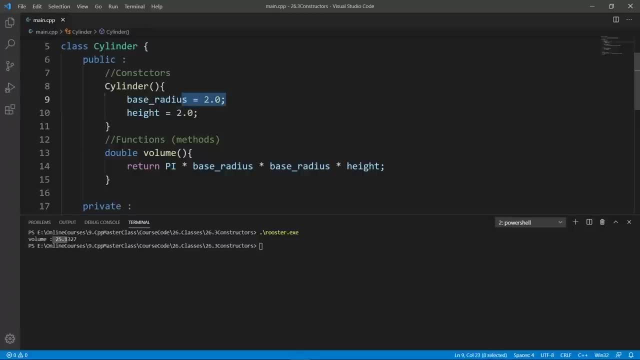 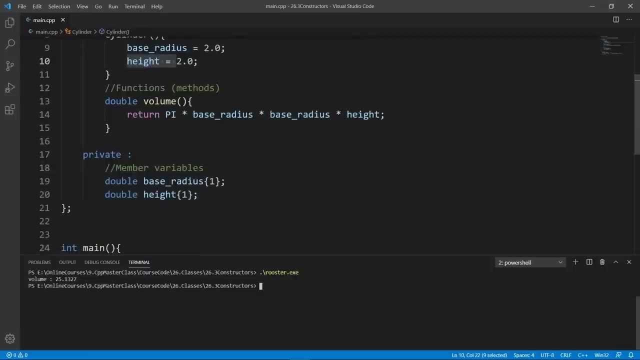 by this base radius, multiply by this base radius again and multiply by height. we're going to get this here. you can try this out. it is going to be what you see here, and this hopefully proves that the compiler is using our constructor here, but we can also use a debugger. let's set up a. 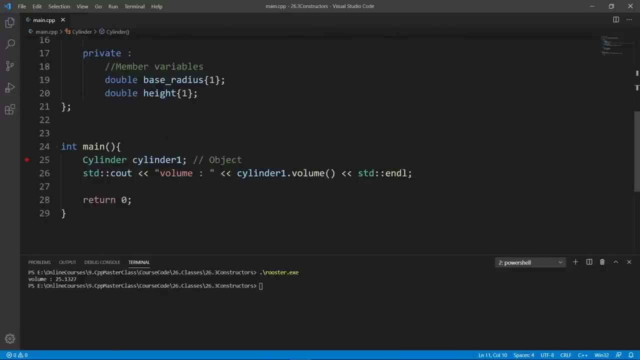 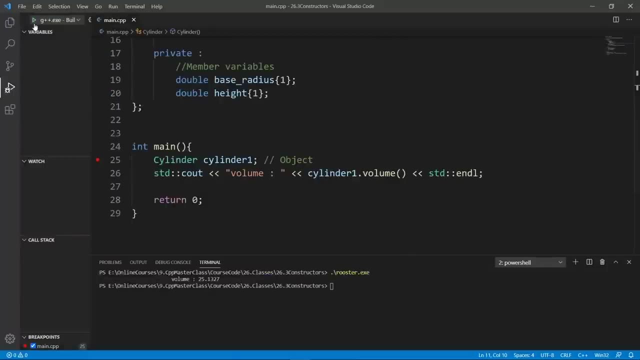 break point here and we're going to run this through our debugger. we can come back to the run tab here, as we have done before, and we're going to try and use the debugging tools that come with the gcc compiler. that's what we can use, if you are. 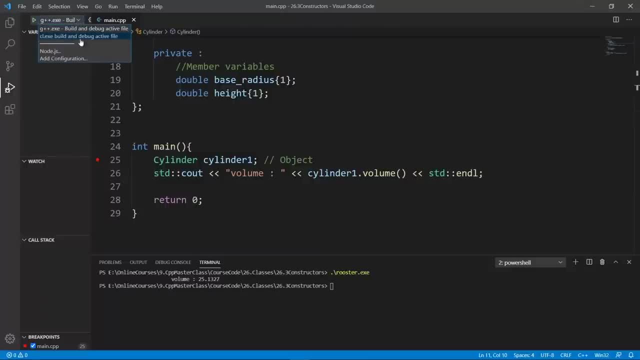 on windows. you can also use the debugging tools that come with the compiler from microsoft, but we're not going to use that now. gcc is going to be fine. we're going to start debugging and we should hit our break point when the build is done. let's wait a minute. okay, we have hit our break. 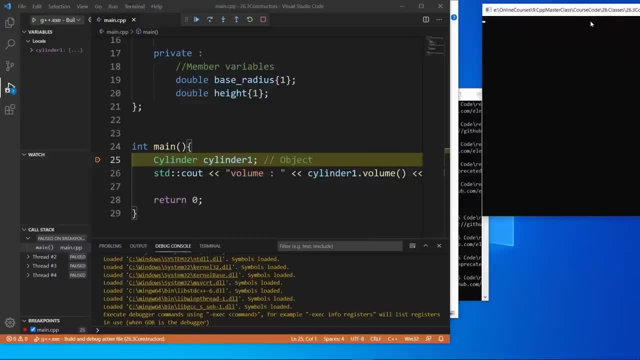 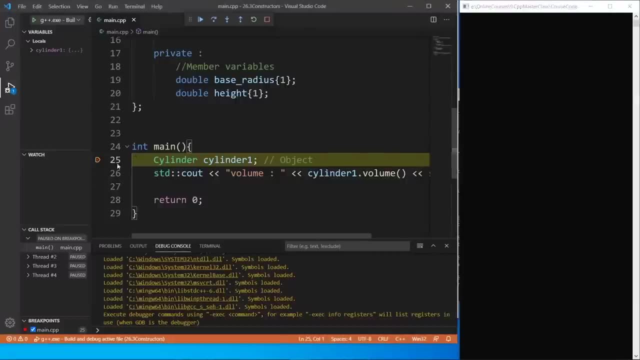 point here. i think we can do that, let's do that. let's put that a little bit to the right here and minimize a little bit. okay, we have our thing in place. we have hit our break point. you see, these are the local variables we have here. we have a cylinder object which is not initialized yet. 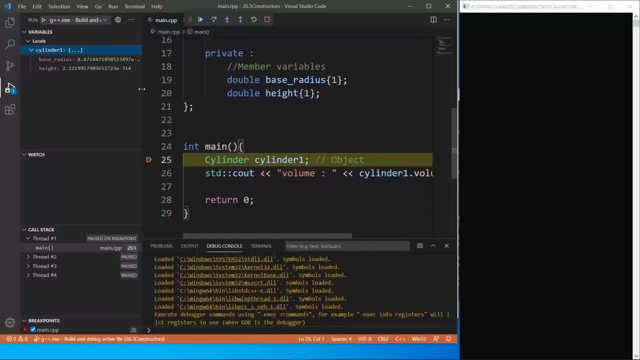 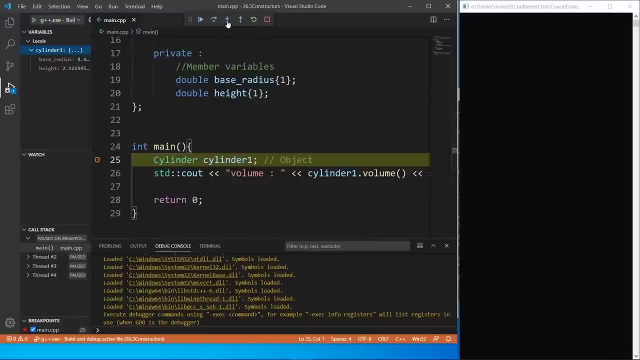 because you see, what we have inside is really junk data. we haven't put in anything yet. but now that we are at this break point here we can hit step into and step into the code that constructs our cylinder object, because at this point line 25 here hasn't run yet. 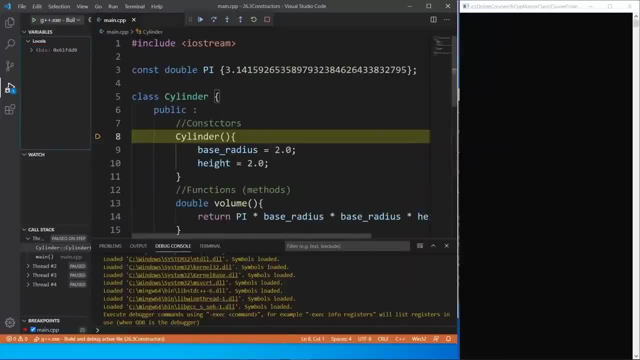 so we're going to step into and you're going to see that we hit the constructor for our cylinder object and this again proves that our constructor is being used to build our cylinder objects. now we can move to the next line. we're going to set up the base radius and if we hit next here, 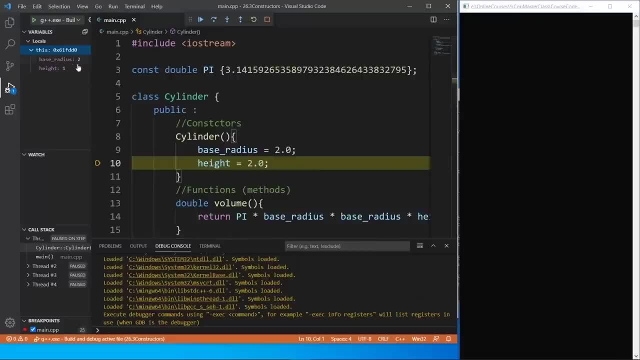 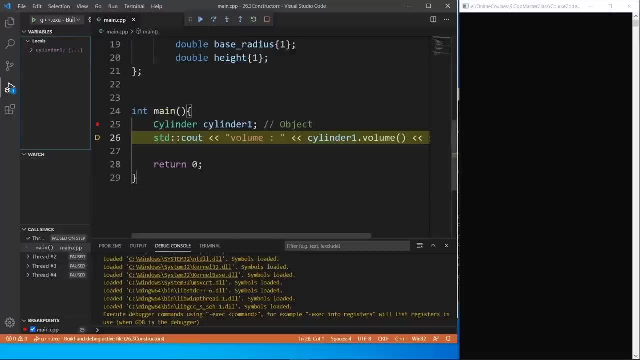 this is going to set our base radius to two, and you see that height is one because we haven't set it up yet. but if we execute this line, you're going to see that height is also going to change to two. and now, if we hit next, we're going to get out of our constructor and our cylinder object will be already constructed. 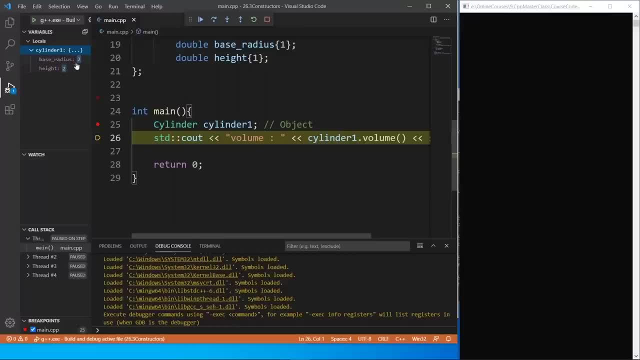 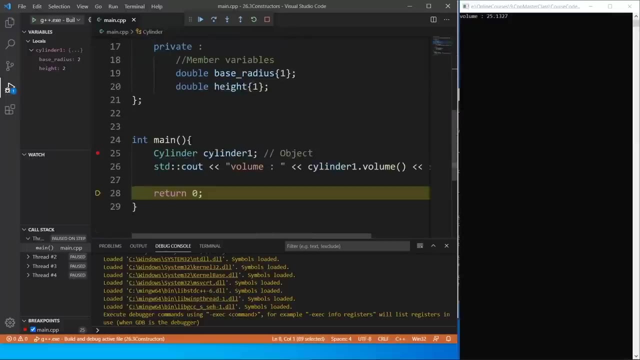 if we look again here, we're going to see that radius is two, height is two and we can print the volume, and if we hit step over, we're going to see our volume printed out here, hopefully. again, this proves that our constructor here is being used to build objects. 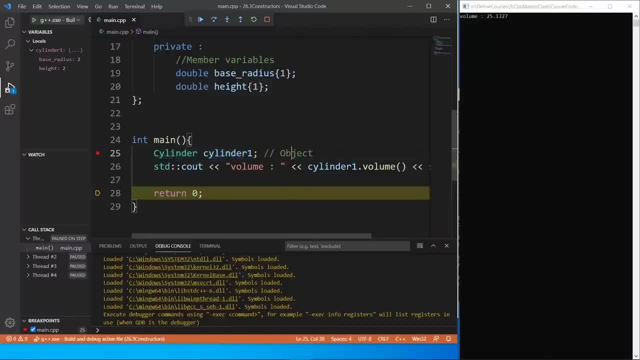 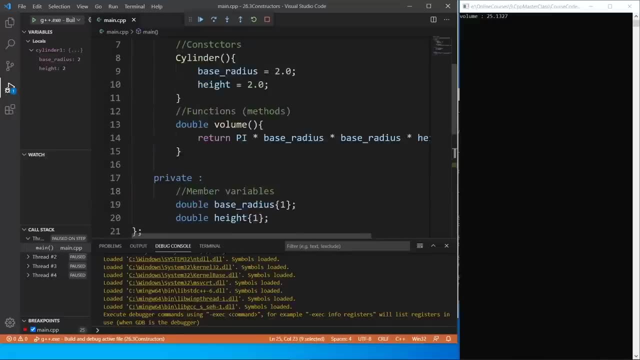 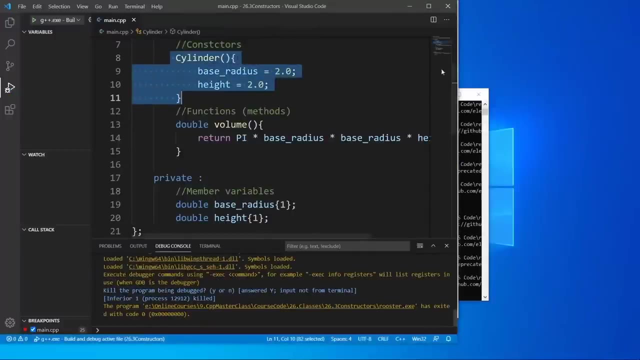 and it is doing that because it sees the syntax here. we don't pass any parameter to our cylinder object as we create it, so this must be calling the default constructor, which doesn't take any parameter. this is the message here. let's close our debugging session and maximize our visual. 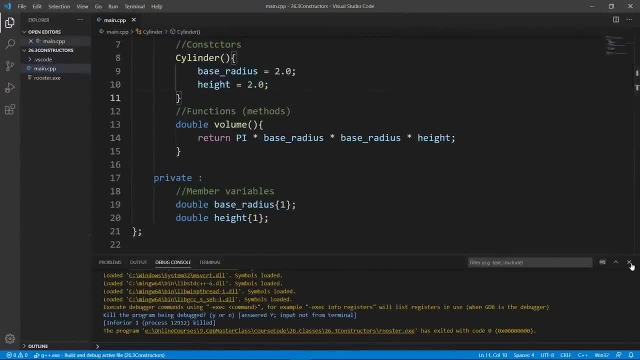 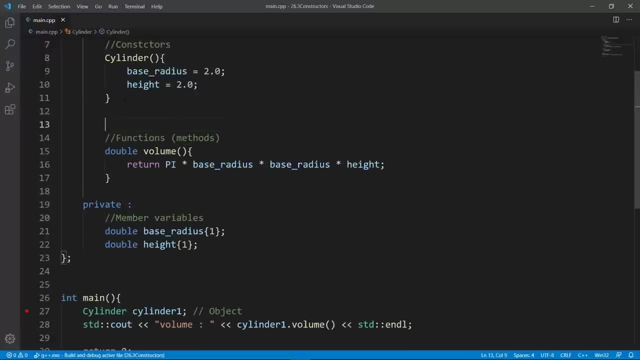 studio code instance, because we're going to set up our cylinder object and we're going to set up our constructor which is going to take parameters. now- and you have seen the syntax to do that in the slides, it is nothing complicated- we're going to say the name of the constructor which is going to 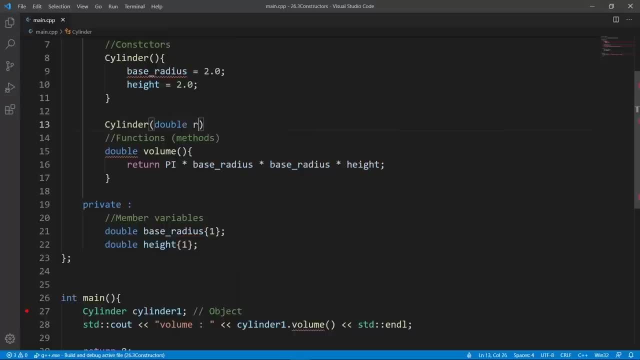 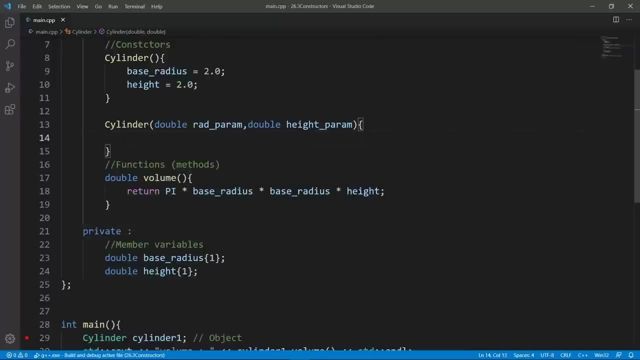 be the name of the class and we're going to say double and say rad param for radius, and we're going to say height param for our height, and we're going to make this double and after that we're going to head in the body of our constructor and we're going to initialize our guys to 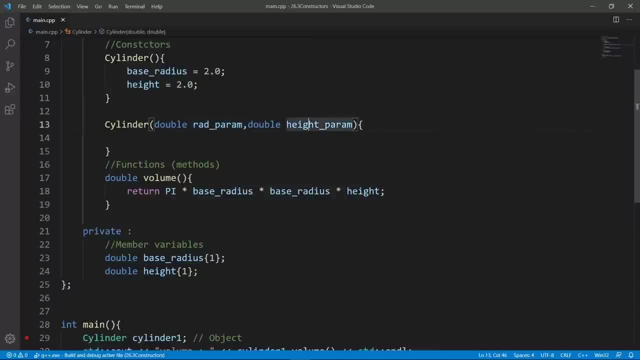 the parameters that will pass to the function here, and this is really powerful after we have this constructor and we will be able to pass parameters that will be used to construct our cylinder object. so we can say base radius and pass in rad param, and we can say height and say 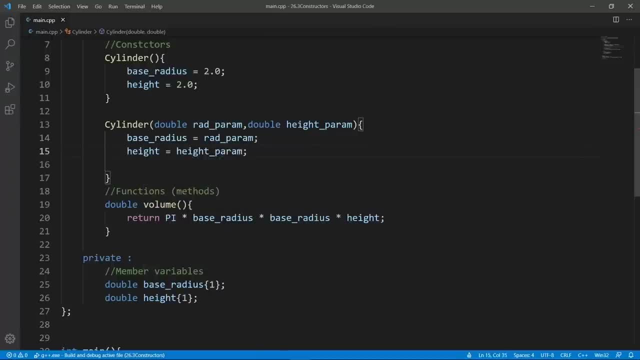 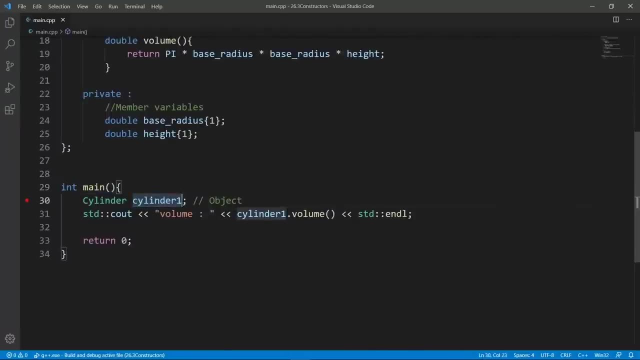 height param here, and these are going to be used to construct our object. now we can head over in the main function and change how we construct our cylinder object. if we want to use 10 as the radius and 5 or 4 as the height, we can do that by passing arguments to our constructor. here let's run this. 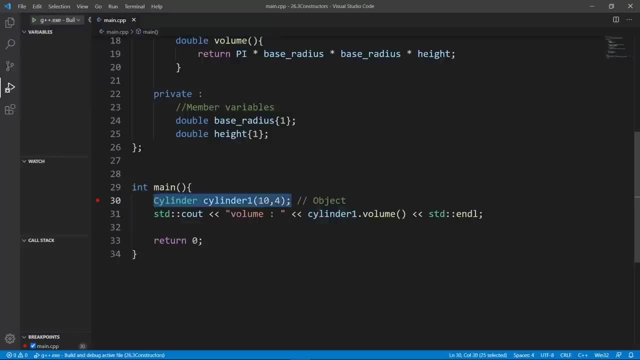 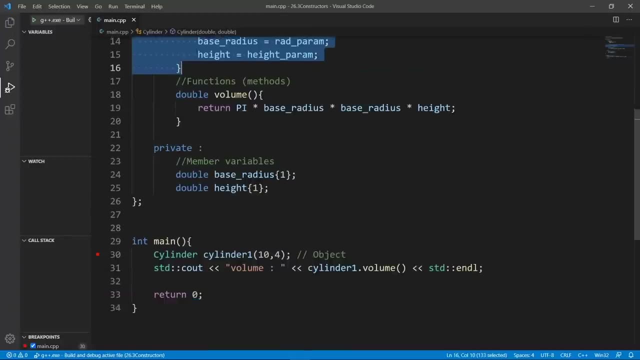 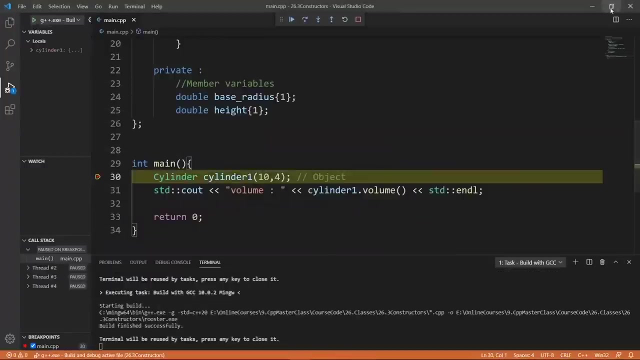 through the debugger again and see that our information here is being used. now this constructor here is going to be chosen by the compiler because it is more fitting for the call that we are doing here. here let's run our debugging session, the program is going to be bolt and we are going to try and. 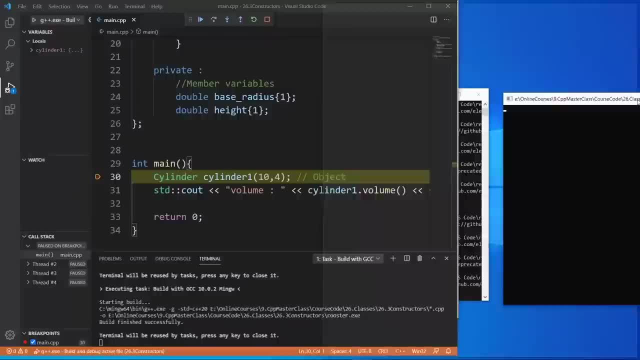 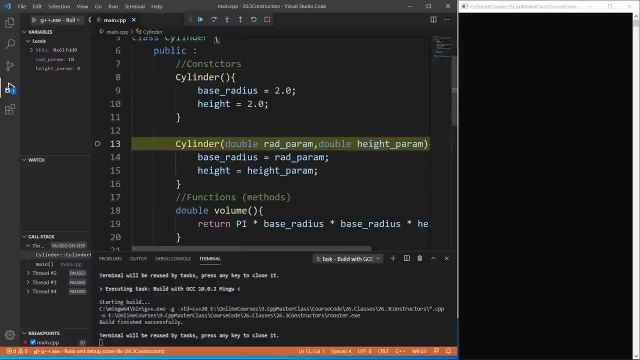 maximize this a little bit and bring up our terminal output. okay, we have hit the break point here. we can step into our constructor and notice the constructor that the compiler chooses. our constructor that takes parameters is chosen here and we can do things inside. let's hit next. 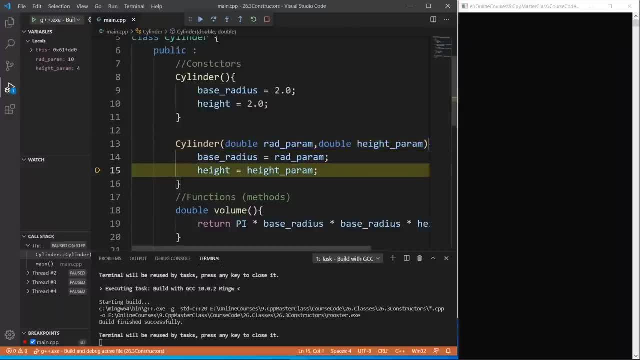 we're going to initialize the base radius to 10 and we're going to initialize the height to 4. okay, we can see that to the left here. if we hit next, the height is going to be changed to 4 and our constructor is going to be done. we're going. 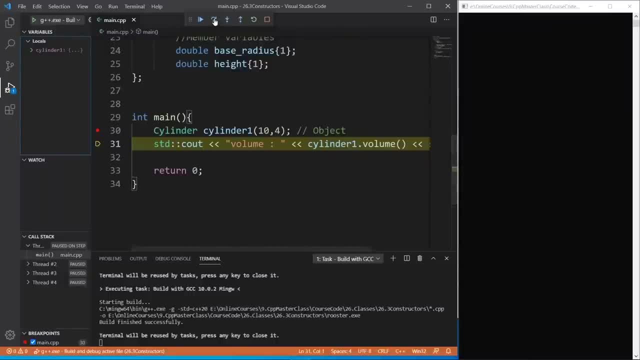 to head over in the main function again, and if we step over now, we're going to print a new volume which is based on the information we use to construct our object. here. this is really what constructors do. they are used by the compiler to build your objects. 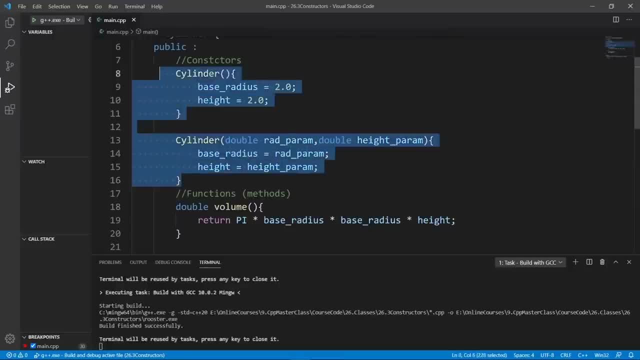 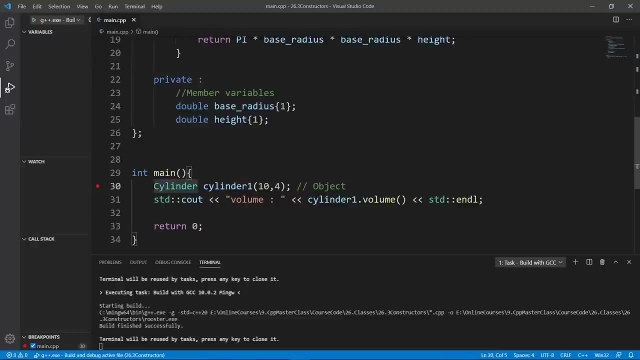 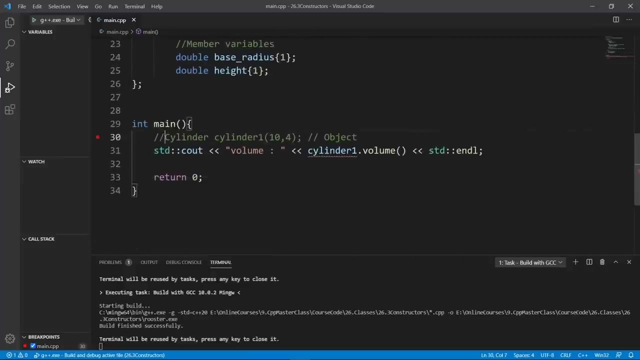 and we saw the syntax we can use to set up constructors for our own classes. okay, now you must be saying: if we need constructors to build our objects, why was the code in the last lecture working? in the last lecture we did something like this. we said cylinder, cylinder one. 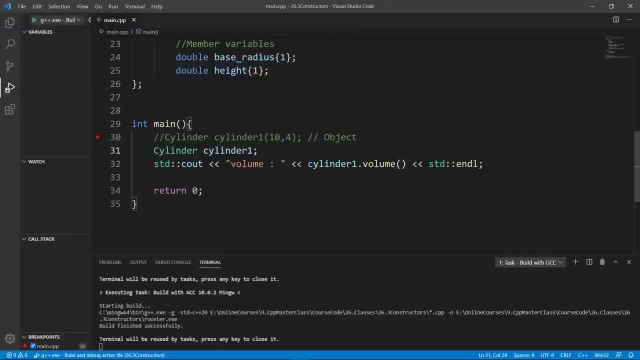 cylinder one, and this was welding and compiling. fine, and let's try and take out our constructors. we can do that. let's comment them out and if we want to set up constructors for our classes, for the less we can, one class for each class and we need to set up constructors for all our classes. 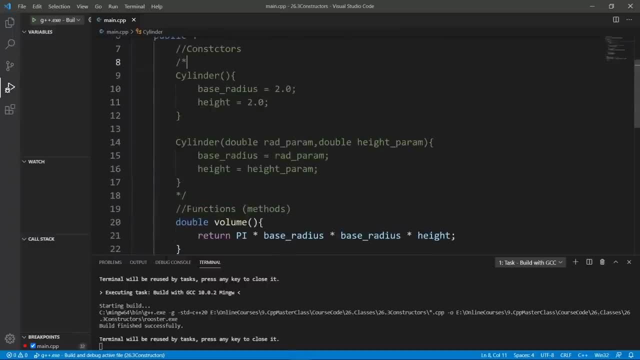 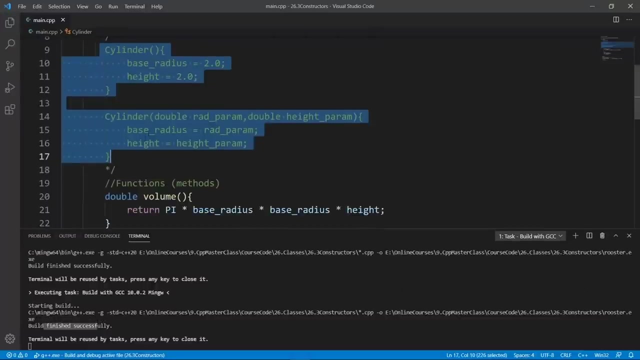 you look, you're going to see that the code is going to compile. fine, even if we don't have any constructors in here. let's build with gcc to show you that the code is going to compile. both is good. so how is this working? how is this constructing our objects, even if we don't have any constructors? 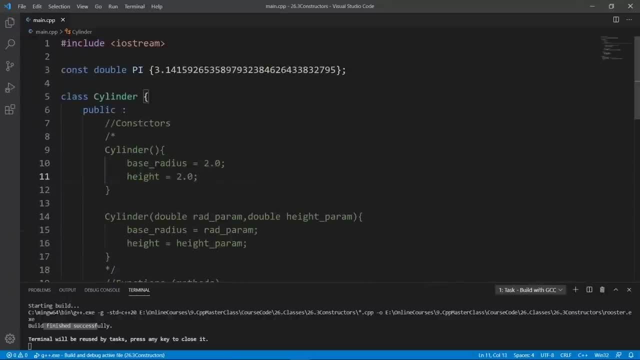 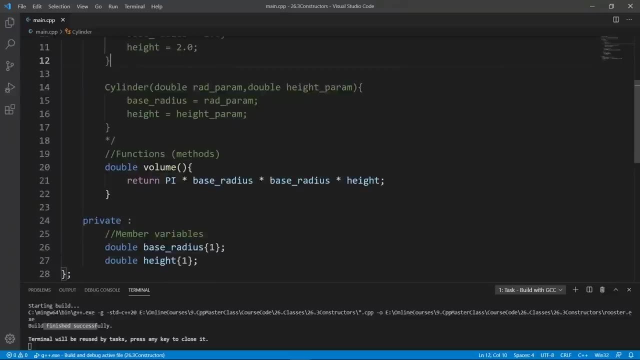 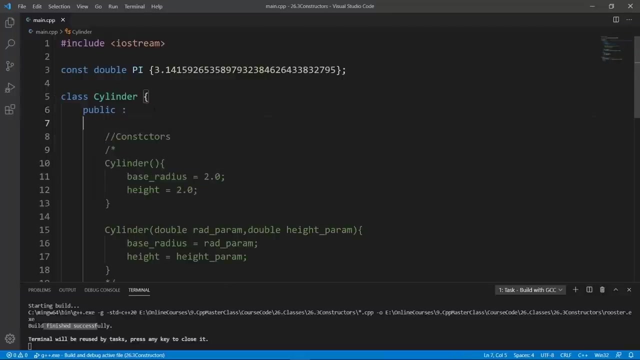 in here. well, the reason is, the compiler is going to set up its own constructor, and what it is going to set up is a constructor which is really empty and doesn't have anything inside. it's basically going to be as if we put in an empty constructor. let's copy this and actually show you this. we can. 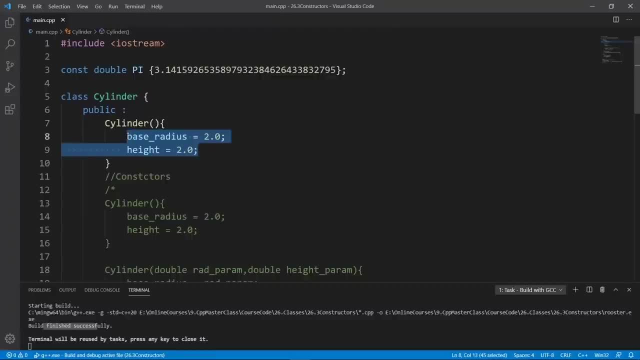 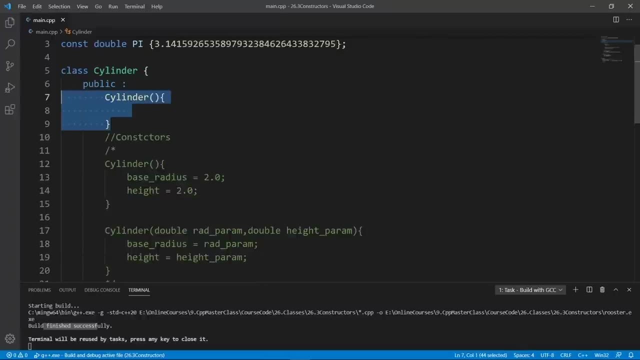 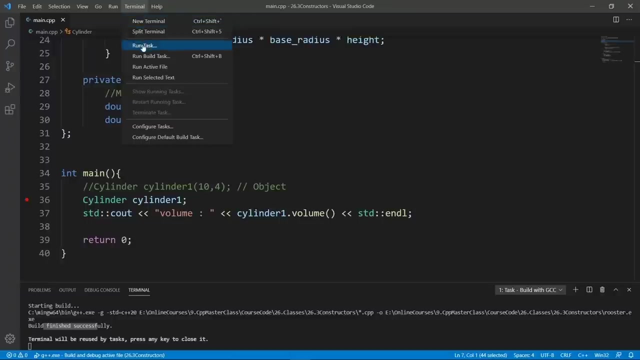 do that and we're going to make this constructor empty and not do anything in the body. this is the constructor that your compiler is going to generate and if we build now and try to set up a breakpoint here, you're going to see that our empty constructor is going to be chosen. let's debug and show you that. okay, you see that we're going to hit. 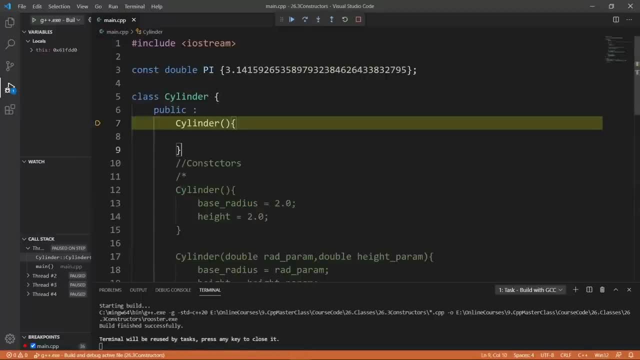 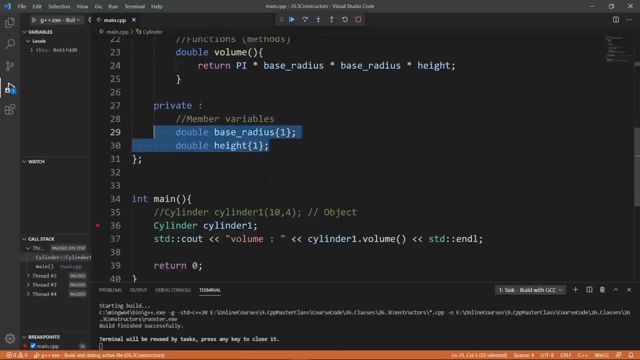 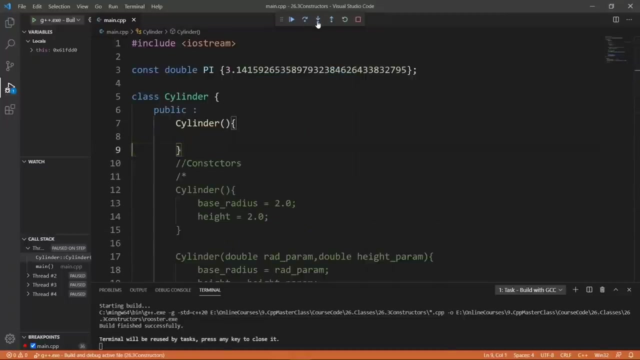 the breakpoint here and if we step into, the compiler is going to choose this guy and it's not going to do anything. so it's basically going to take our member variables as they are and it's going to use the information to print the volume. here we can hit next again and get out of our 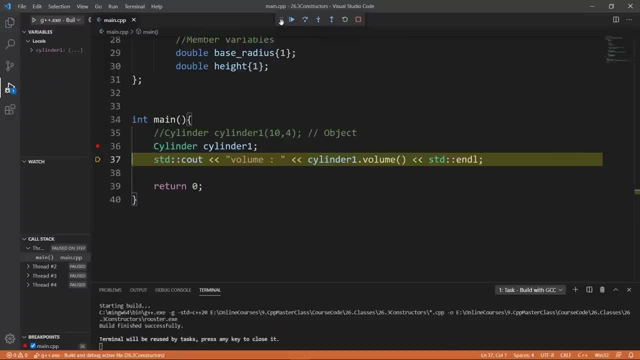 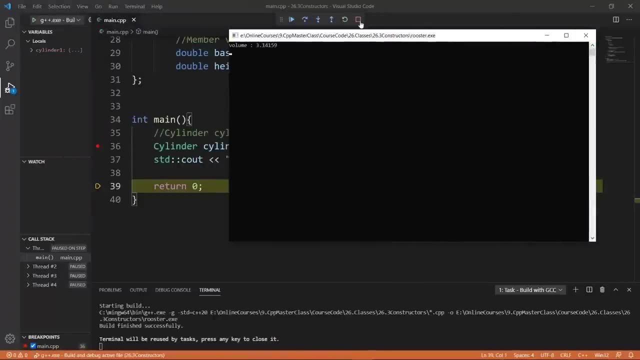 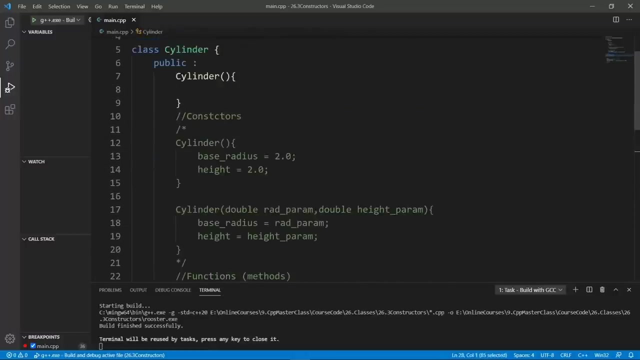 constructor and if we step over, we should print our volume, which is going to be 3.14, because the compiler just used the initial values we have in our member variables here. so again, the message is: if you don't have any constructor in your class, the compiler is going to generate an empty constructor for you and the empty constructor 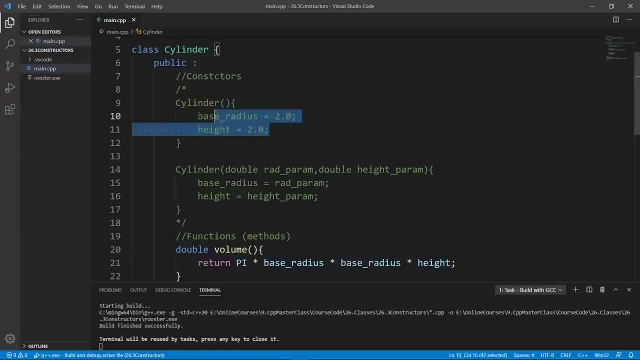 is going to take no parameters and it's not going to have anything in the body. it's going to be an empty constructor and it is called an empty constructor. and it is called an empty constructor- default constructor generated by the compiler. this is really all i had to share in this lecture. 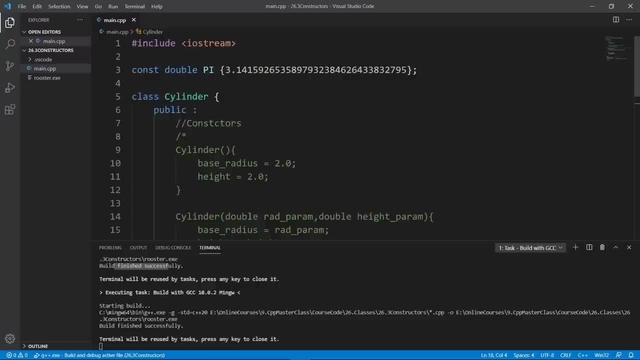 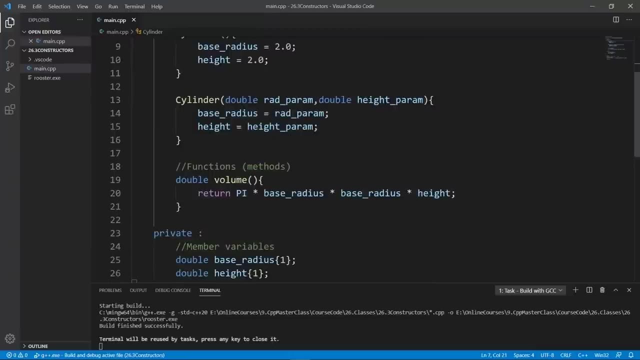 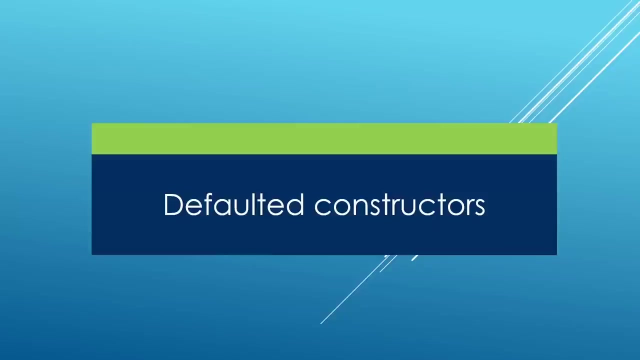 i hope you found it interesting. now you should have enough knowledge to build your own constructors for your classes. we are going to stop here in this lecture. the next one we're going to learn about default constructors. go ahead and finish up here and meet me there. in this lecture, we're going to 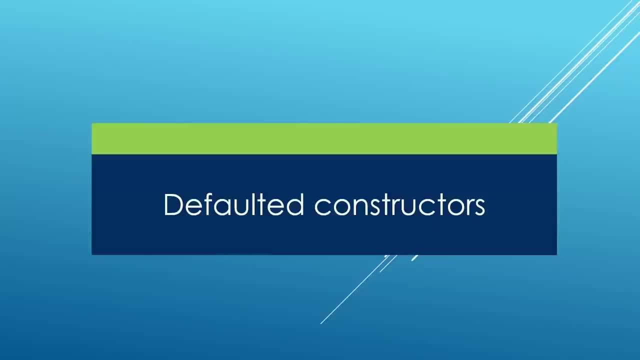 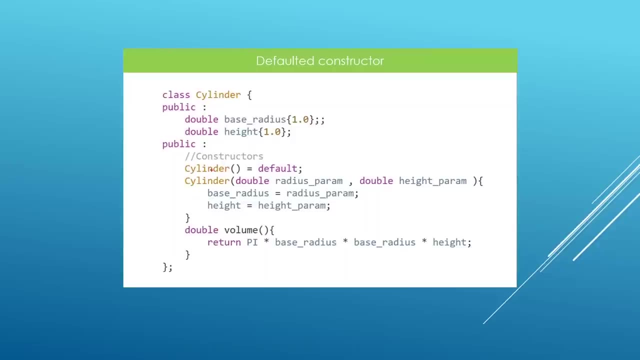 learn about default constructors, and this is a syntax you can use to let the compiler generate a default constructor for you. all you have to do is do things like this: you're going to say the name of the constructor, which is going to be the same name as the class. you're going to 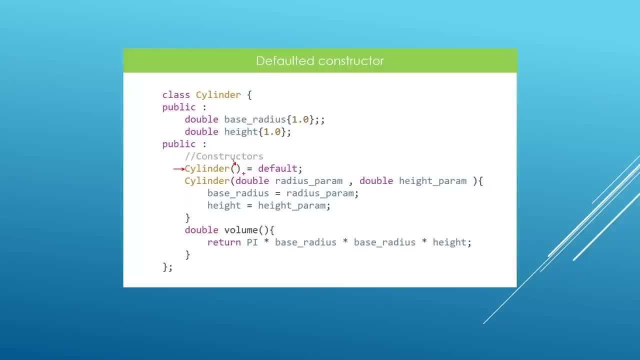 put in an empty parameter list and then you're going to say equals default. if you do this, the compiler is going to generate a default empty constructor for you. in the last lecture, we have seen that we can set up our own constructors, basically like this: what i haven't told you. 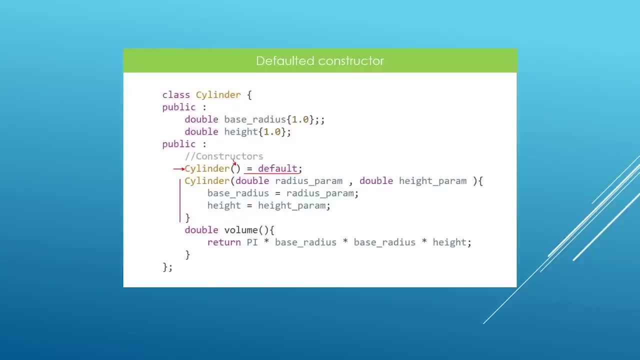 is that the moment you set up your own constructor, the compiler is going to not generate the default constructor, and if you want to keep the ability to construct objects without passing parameters, you're going to have to put in your own default constructor, and you can use this syntax here. 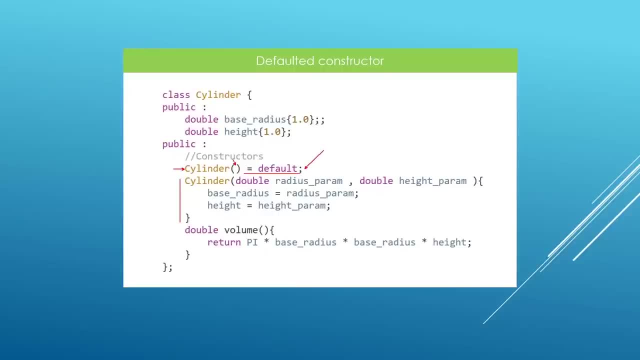 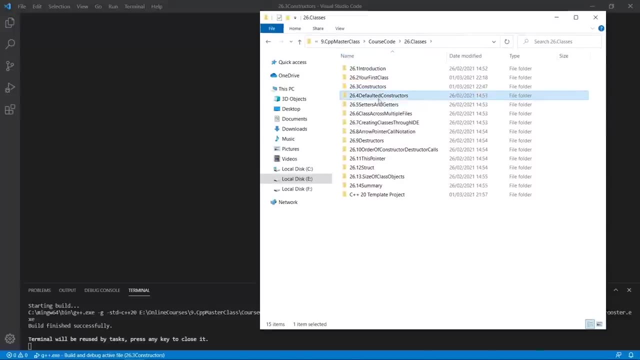 to do that, let's head over to visual studio code and talk about this a little more. okay, here we are in our working folder. the current project is defaulted constructors. we're going to grab our template files and we're going to put them in place, and we are going to open this in visual studio code by: 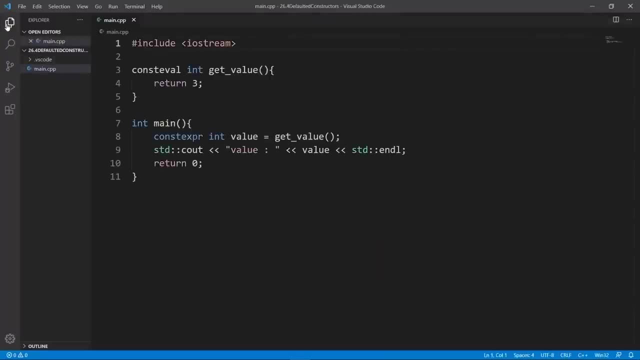 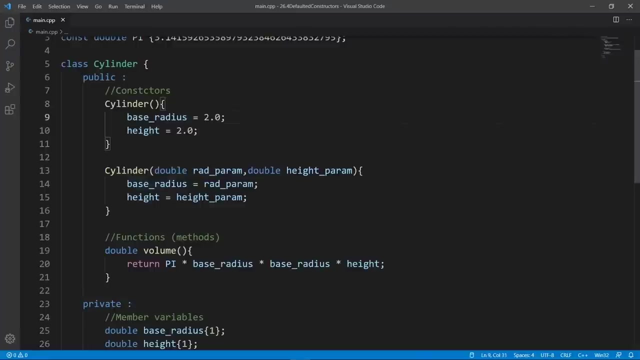 dragging and dropping here and we're going to open our main CPP file. let's take out what we don't need. we're going to clean the main function here and we are going to bring in the class definition we had in the last lecture. if you remember, we had two constructors and one constructor which didn't take any. 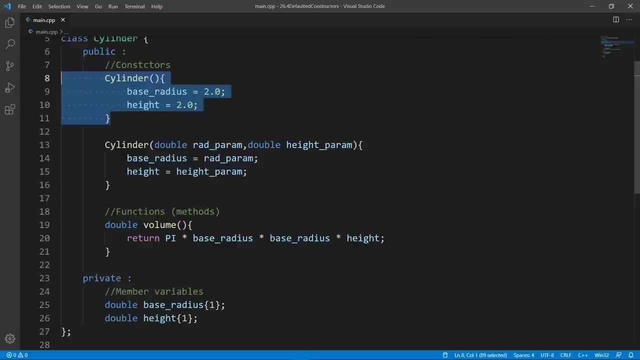 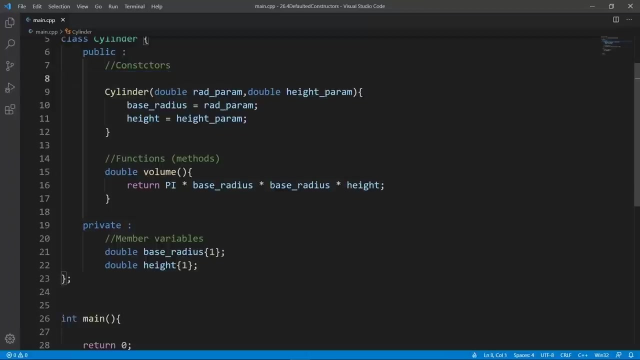 parameter and another constructor which was initializing our member variables with parameters that we pass in this parameter list here. but in this lecture let's take out this constructor that doesn't take any parameter and show you that when you set up your own constructor, the compiler is not going to. 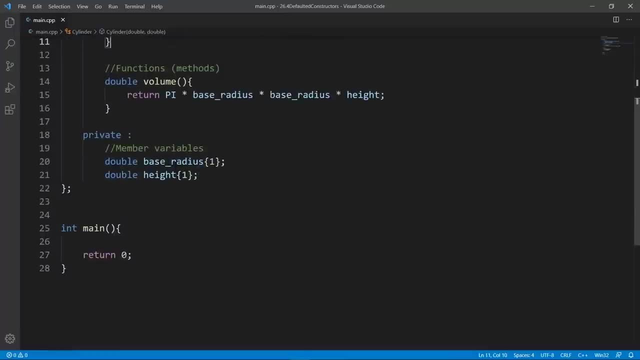 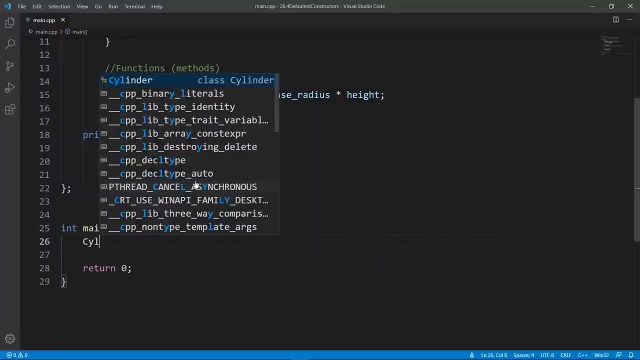 generate a default constructor for you and we're going to lose the ability to construct objects without passing parameters. the syntax you basically see here: we're going to say cylinder and say cylinder one. let's use a lowercase C and if we do this, you see that we have a. 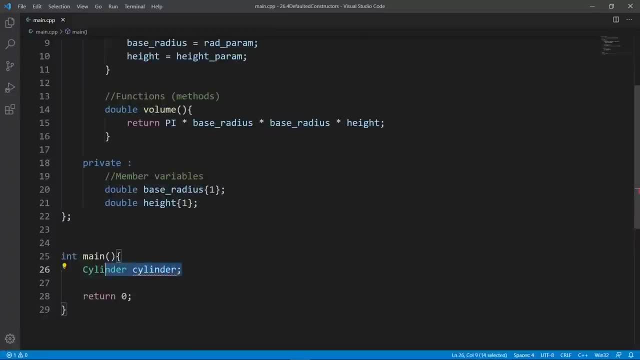 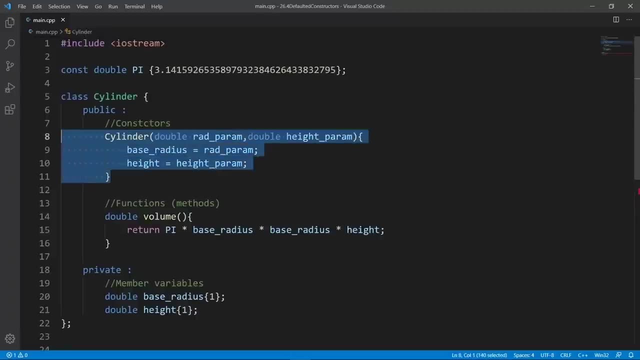 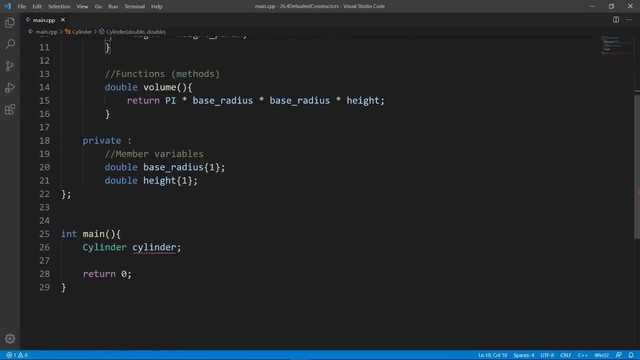 squiggly line. the compiler is not going to generate an empty, non parameter, taking a constructor, because it sees that we have a constructor view. this is how C++ compilers work. if they see that you have any constructor in your class, they're not going to generate a default empty constructor. and if we're trying to 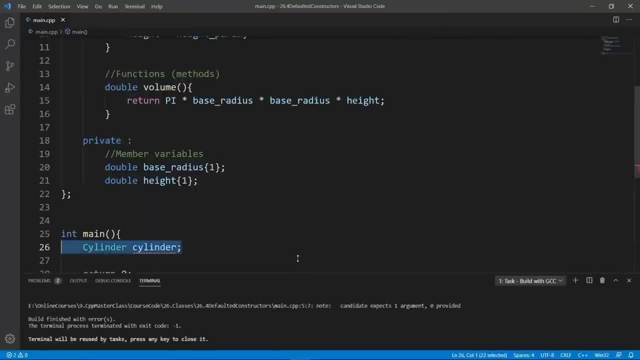 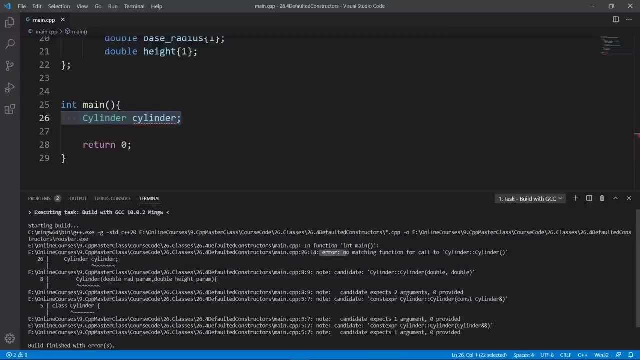 work with a constructor. we're going to have a constructor that is going to be world. we're going to get an error that says something like: we don't have a constructor that can basically construct an object from the line. here it's going to say: no matching function, call for cylinder, cylinder. you see, here it is. 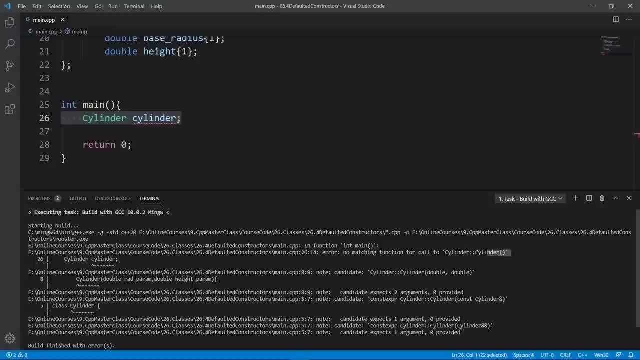 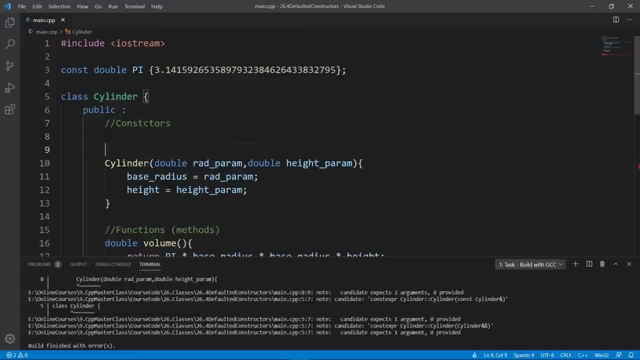 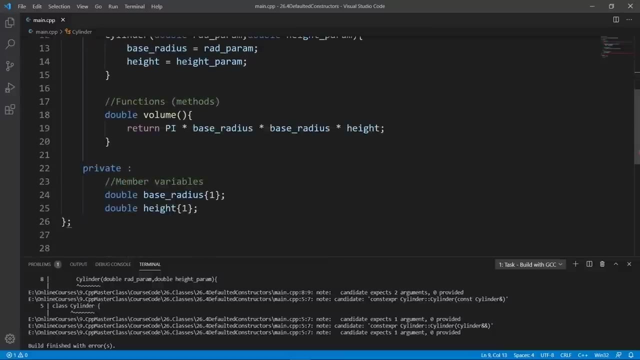 trying to call a constructor that doesn't take any parameter. but we have no such constructor in our code. we could go in and put in that constructor and, for example, say cylinder, and put an empty parameter list and put an empty body. now this line here is going to work because we have a default empty. 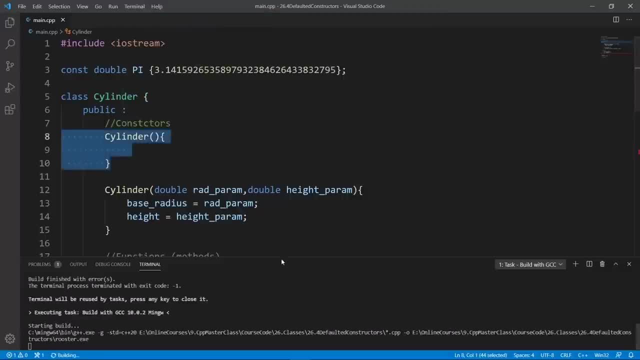 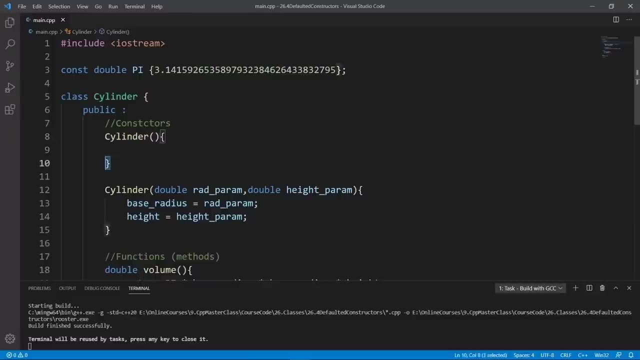 constructor and if we world, you see that the world is going to be good, okay, we are building, fine. but having to type all this, if what you really want is an empty constructor, is too much type in, and in C++ we have a syntax we can use to let. 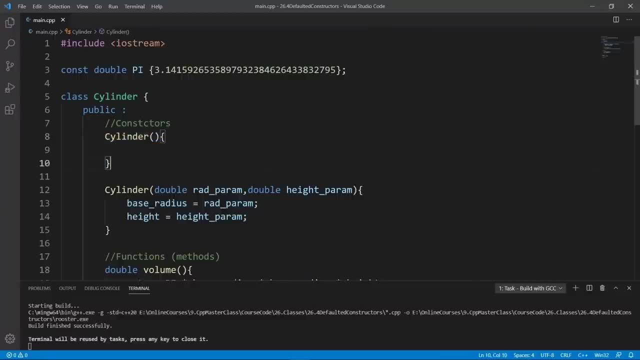 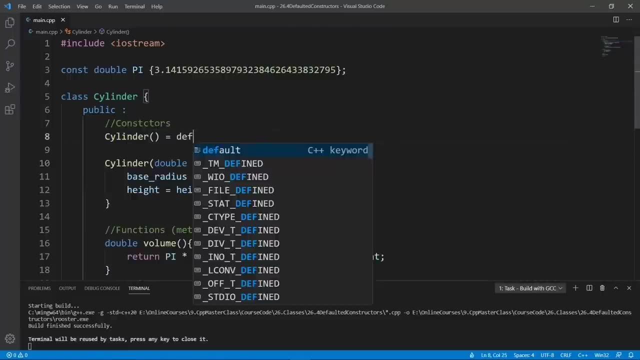 the compiler generate this kind of constructor for us, and the way we do that is say cylinder, and then we're going to say cylinder, and then we're going to say constructor, and then we say the name of the constructor, we say equals and we say default. if we save this, the compiler is going to generate this. 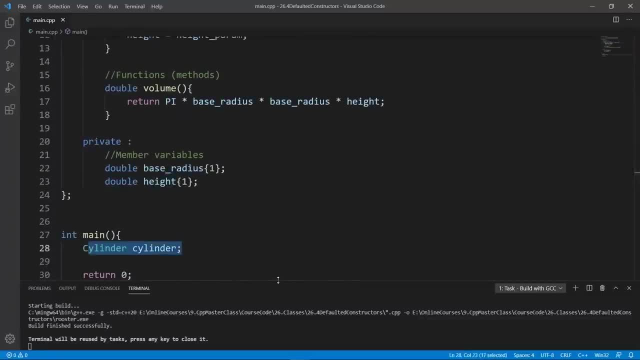 constructor for us and the line here is going to work, so let's bring this up and build again. we're going to build with gcc. you're going to see that the build is good and we can bring up a terminal and clear and run rooster. we're not going to. 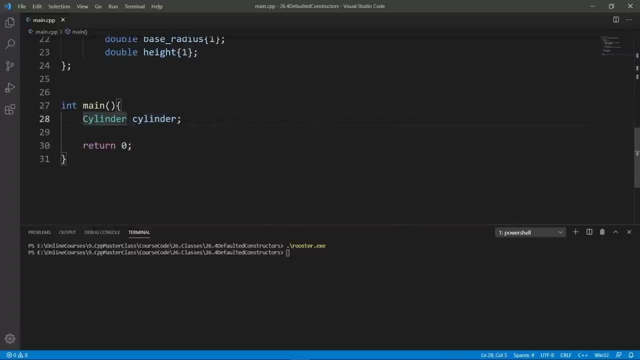 see anything because we're not printing the volume of our cylinder here. but we can do that. let's call this cylinder one, to be consistent with what we did in the last few lectures, and we're going to say stdc out and print the volume of this cylinder. we're going 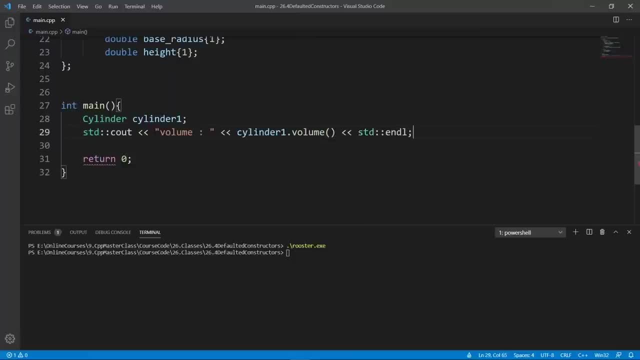 to say volume and call our volume method and now that we have this, we can world. we're going to use gcc to do that. the both is good. we can go down and clear and run rooster. we're going to see that. we see our volume here and this is. 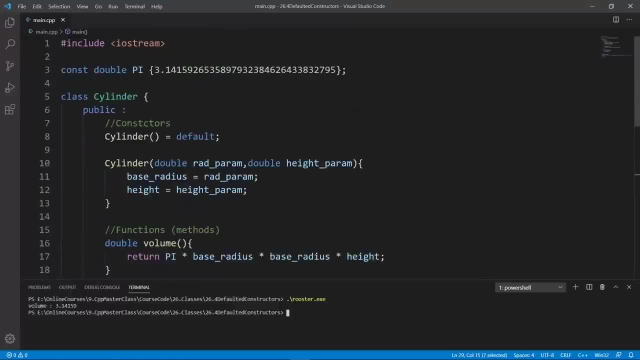 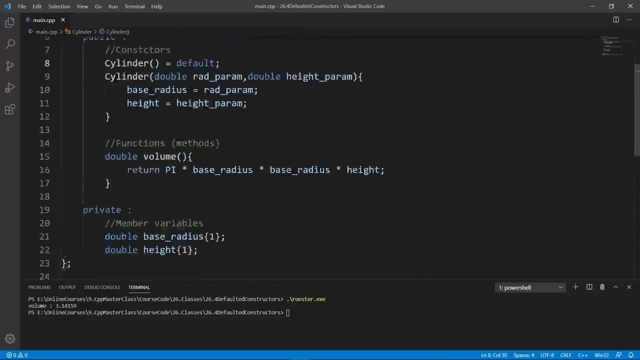 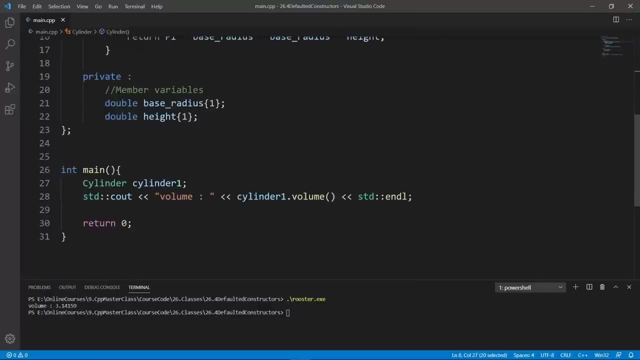 really all I wanted to share with you in this lecture that you can use this default syntax here. so let's go ahead and create an empty default constructor for your classes, and one thing I haven't shown you is that your constructors have to be public to be able to be called like this. and to show you that, let's go up and actually. 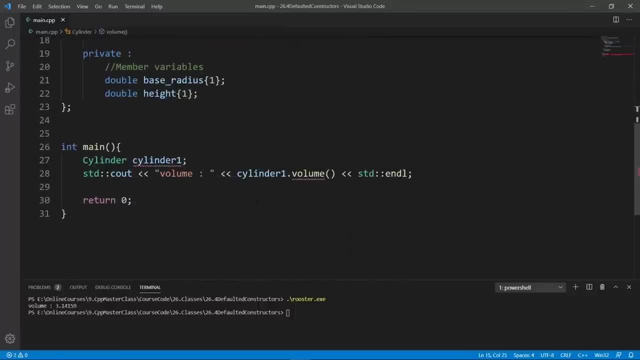 change this to private and show you what happens. the moment we do this, we're going to get a squiggly line in the main function here and if we're trying to build, but before we build, let's show you what Visual Studio codes is saying it's. 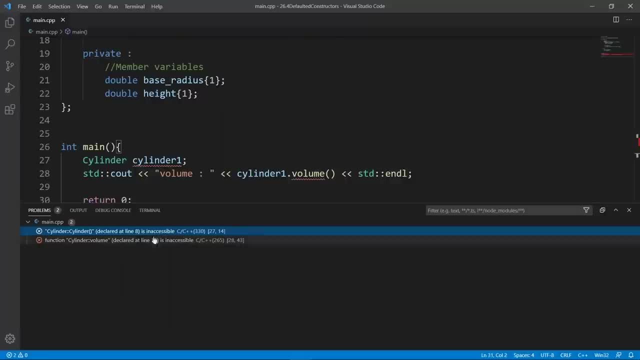 going to say cylinder. cylinder declared is inaccessible. so you see, the constructor which is declared inside our class as private, is it accessible from the outside when we try to call it to build our cylinder objects? so for constructors to be usable on the outside here and build your objects, they have to be public. let's 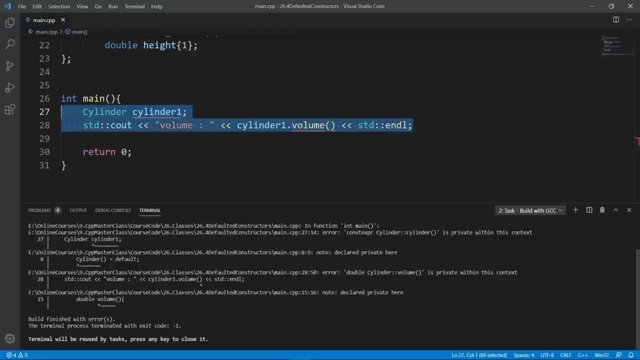 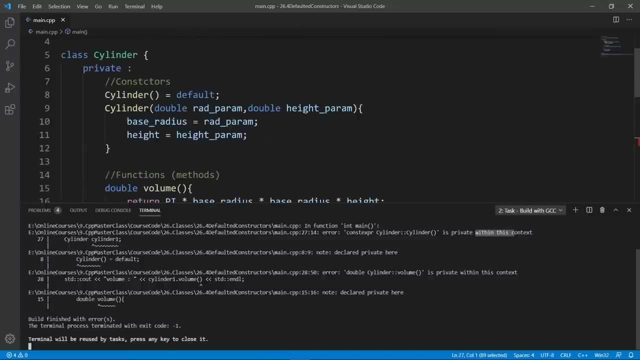 build and see what gcc says about this, we're basically going to have the same error. the constructor is private within context, so we can't really call it. so if we want our code to build, we need to make our constructors public, and this is something you need to know. let's build them and see that the code is now. 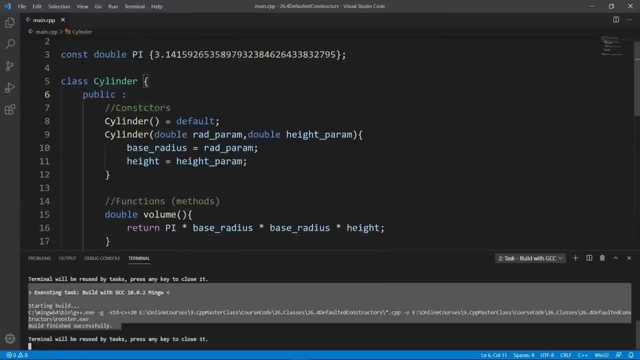 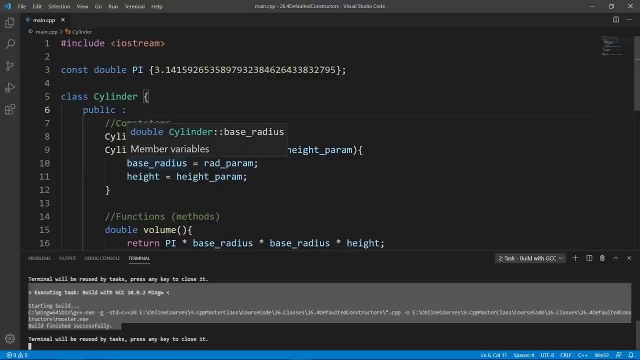 building the world is good, and this is really all i had to share in this lecture. we are going to stop here in this one. in the next one we're going to see how we can use setters and gators to modify things about our class objects. go ahead and finish up here and meet me there. 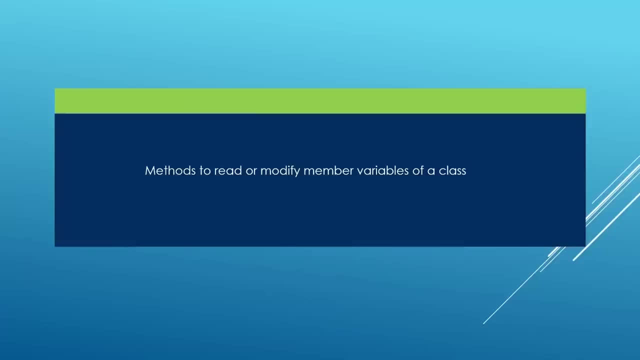 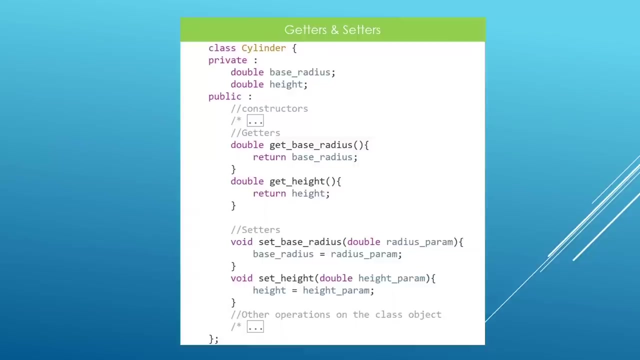 in this lecture we're going to learn about satyrs and gators, and these are methods in our class that we can use to read member variables or modify data in our member variables. let's look at a simple example- and, by the way, i am sorry for my bad pronunciation of cylinder here. i have said it. 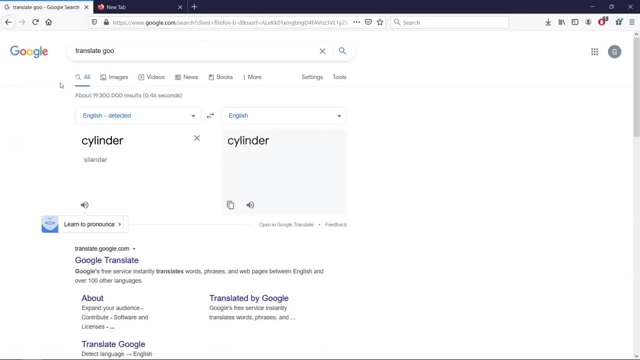 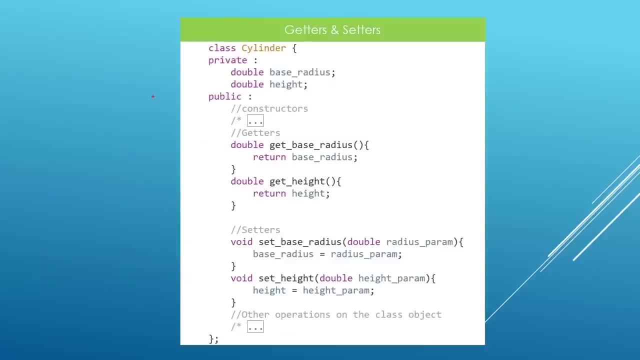 was cylinder and, after some careful thought, i checked online for the pronunciation of this and i found that it was cylinder. sorry for this if it was bothering you. i apologize for the bad pronunciation and i am going to do this right starting from now. okay, here we have our cylinder class, we have a few member variables and we have 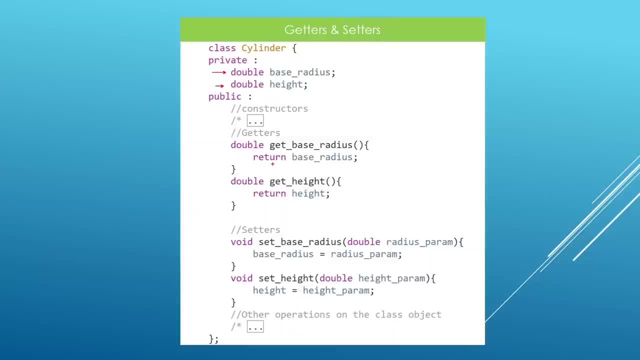 the base radius, we have the height, and now we want to go through some public functions to do operations on these member variables, because now that they are private we can't really modify them or manipulate them from the outside and we really need to do things with them. so if we want to read 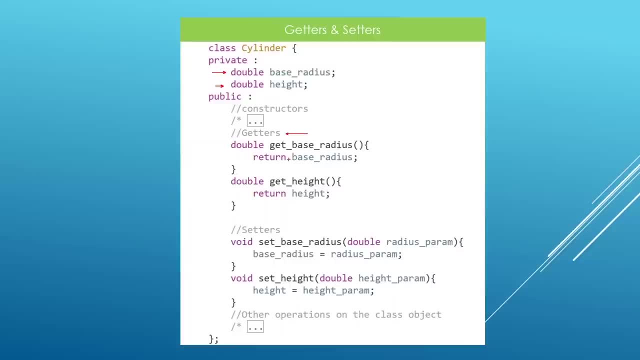 things from them. we will use the gator functions and if you look here, this is a simple function. the only special thing about it is that it lives inside the class, it has a return value, it has a function name, it has a parameter list and then the body we're just going to return. 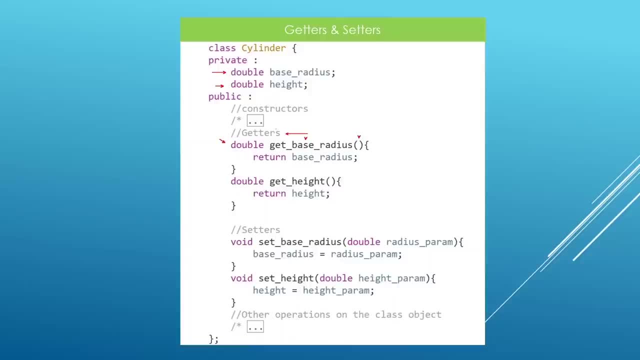 the member variable of interest because this is a getter. we use it to get stuff from the class. this is the meaning here. here we have another getter function which is going to return the height, and notice that these functions live in the public scope of our class. this is key because we want to 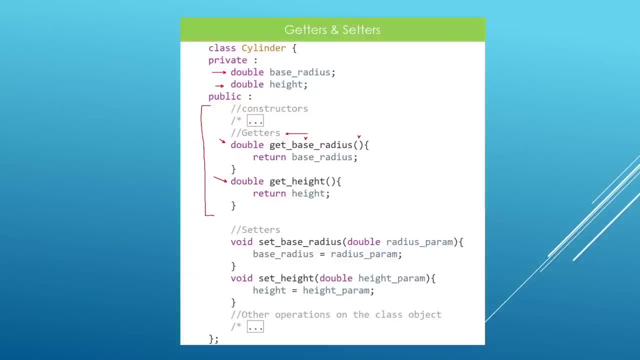 be able to go through them to modify and do things with our member variables, but they will be used from the outside, so they must be public, otherwise they won't be accessible from the outside. we also have a pair of setter functions. they are going to be modifying our member variables, so set base. 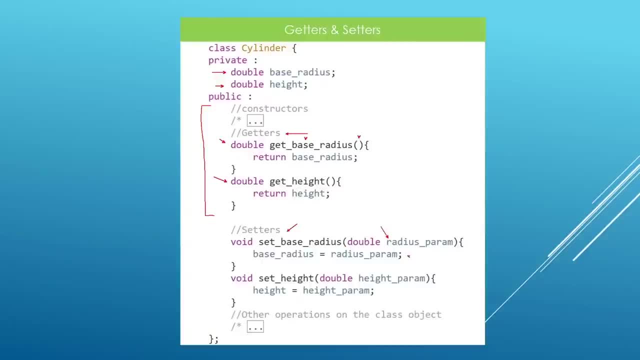 radius is going to take a parameter that it's going to use to set our base radius. set height is going to do the same. it's going to take a parameter and it's going to use that to assign a value to our height member variable. here, and because these functions are members of the class, 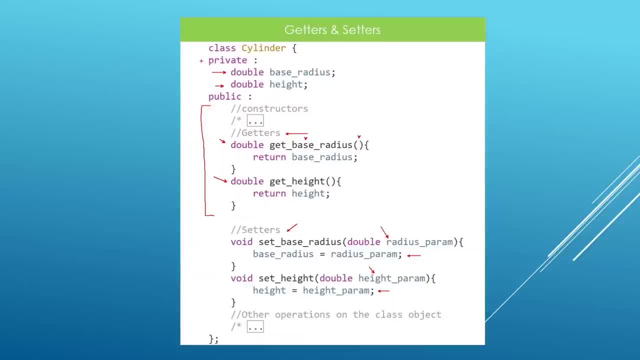 they have access to our member variables, regardless of whether they are public or private. so this is going to work. we're going to go through them from the outside and they are going to do the dirty work for us and do things using our member variables, to which we 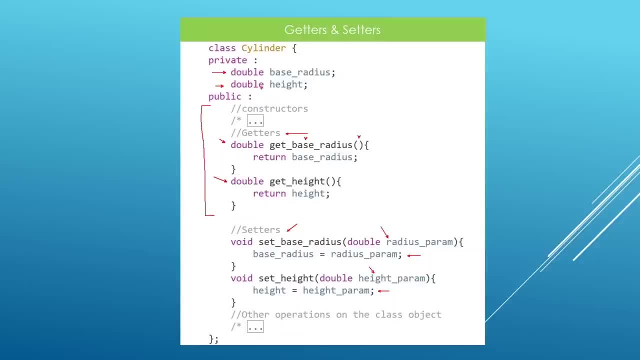 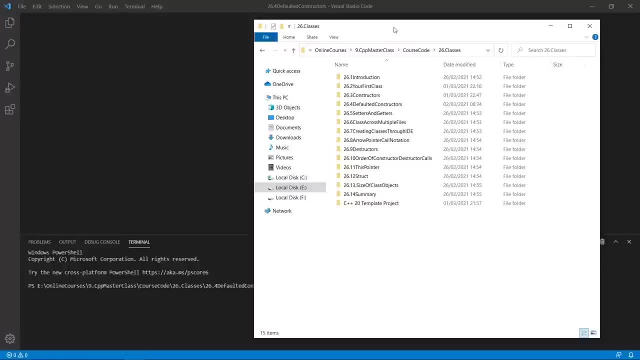 don't have access to from the outside. this is the meaning here. now that you have an idea about this, we're going to head over to visual studio code and play with this a little more. okay, here we are in our working folder. the current project is setters and getters. we're going to grab our 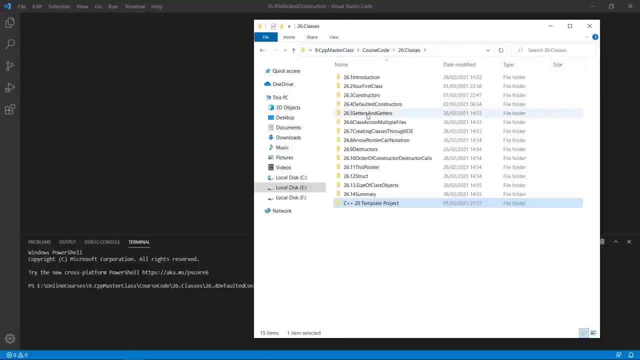 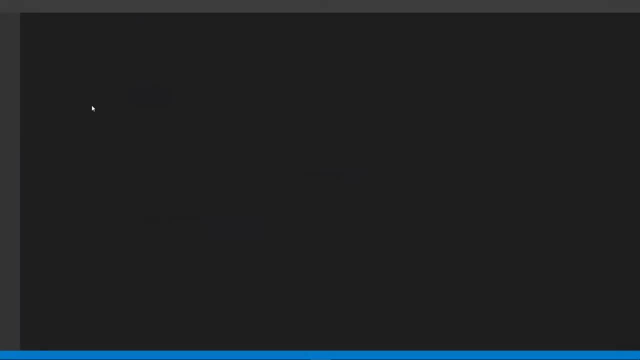 template file and we're going to go to our project and we're going to go to our project and we're going to drag and drop these files pretty quick and put them in place. setters and getters. it is: let's grab the folder and we're going to open this in visual studio code by dragging and dropping here. 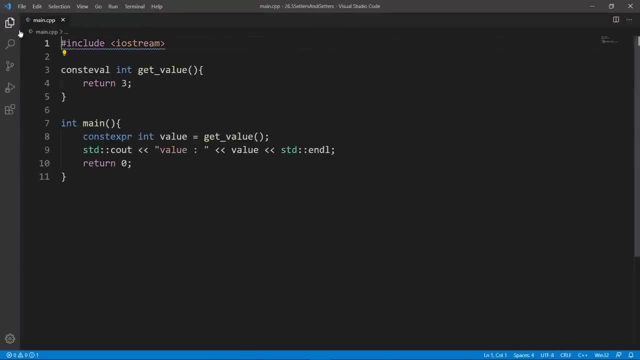 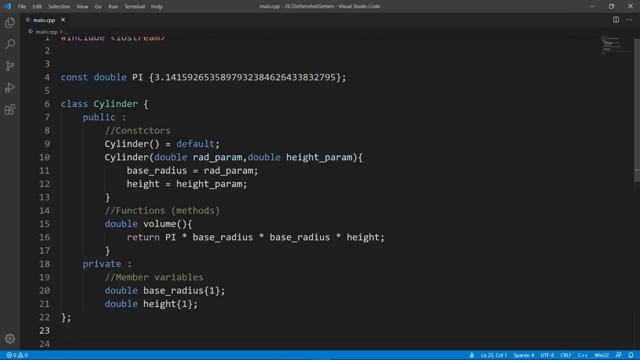 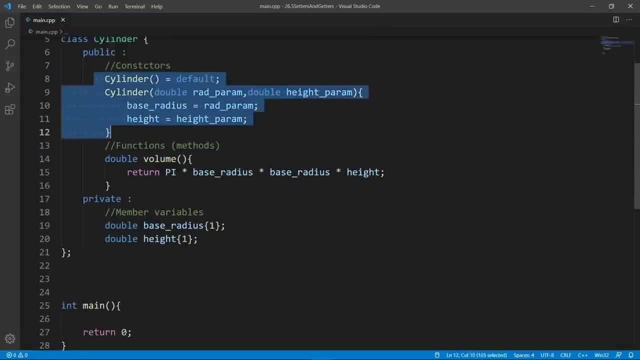 this is going to open our folder. we're going to open our main cpp file and we're going to clean it up a little bit. we are going to grab the cylinder class from our previous lecture and use that as a starting point here. and if you look, we have a pair of constructors here. we have the 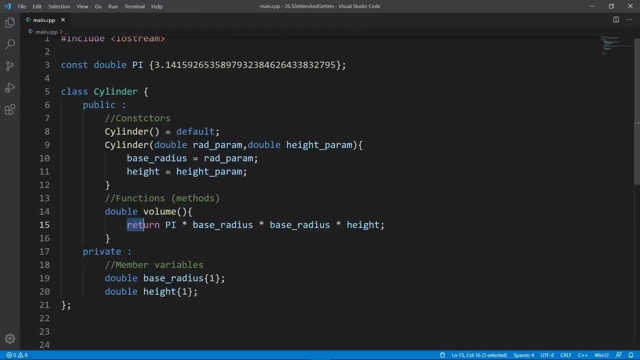 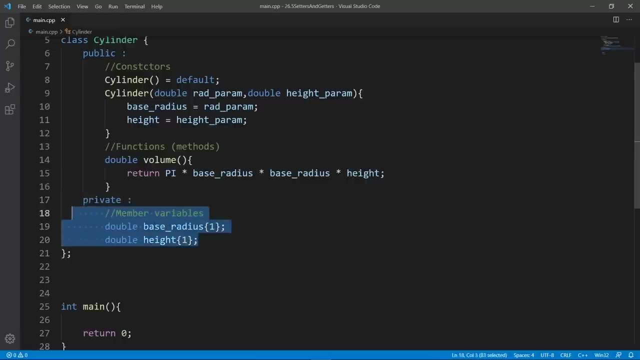 volume function, which is going to do the same thing. we're going to do the same thing here and give us the volume of our cylinder here and we have our member variables. now what we want to do is to be able to do things with these member variables from the outside in the main function. 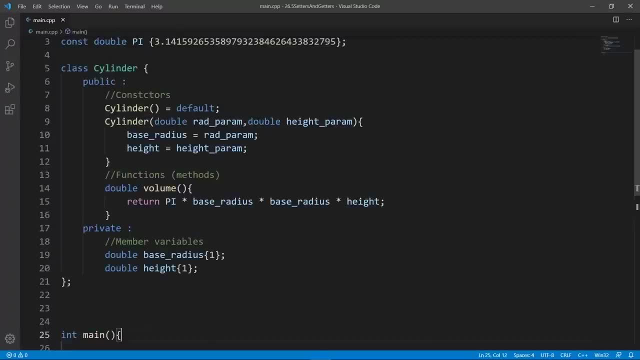 here and we're going to go through setter and getter methods which must be public. so let's do that. so we're going to set up our getter first. so we're going to say: double get base radius, it's going to return double, it's not going to take anything. and and in the body, we're just going to. 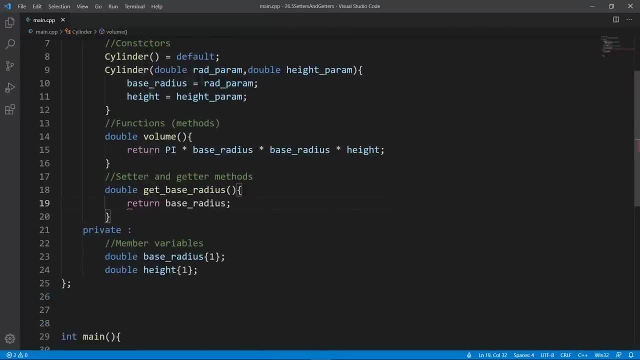 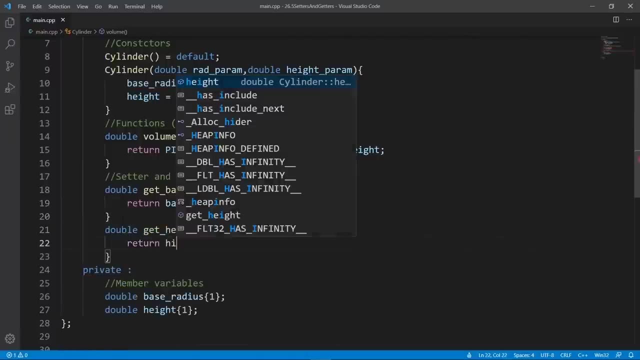 return our radius. let's return that. okay, so we're going to set up another getter which is going to give us the height and it's not going to take anything in, it's going to just return our height member variable. now, these are our getters. they are going to be getting vents from the class object. 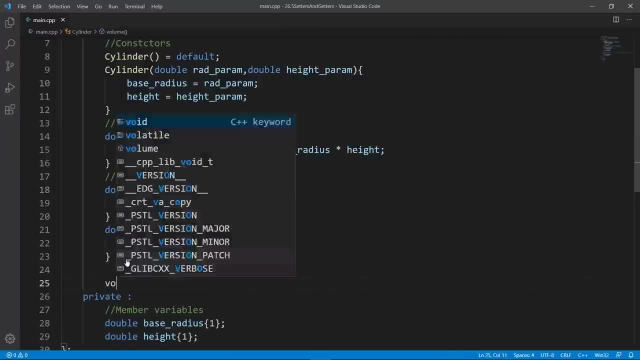 we're going to set up other functions that are going to be our setters. they're not going to return anything and we're going to say set base radius and it's going to take a double parameter in and we're going to use that to set our base radius. so we're going to say base radius and we're going to say equals rad param. 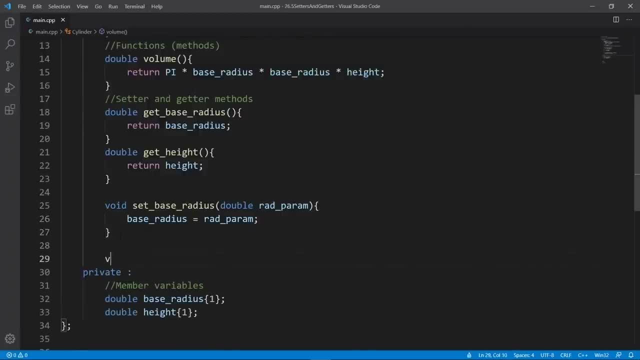 here and we're going to do the same for our height. so it's not going to return anything. the function here, and we're going to say set height and we're going to take our parameter n, so we're going to say double height param and we're going to use that to assign stuff to our 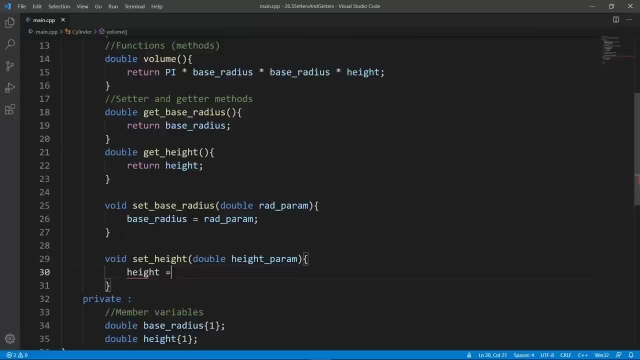 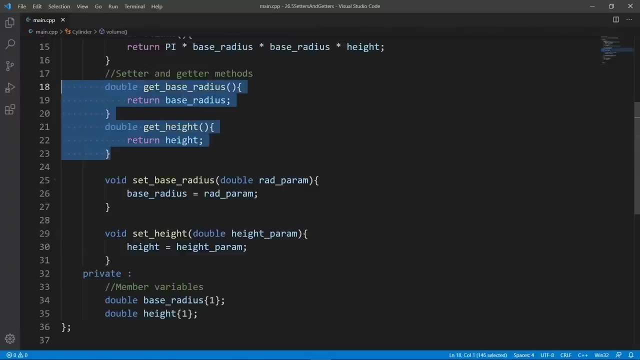 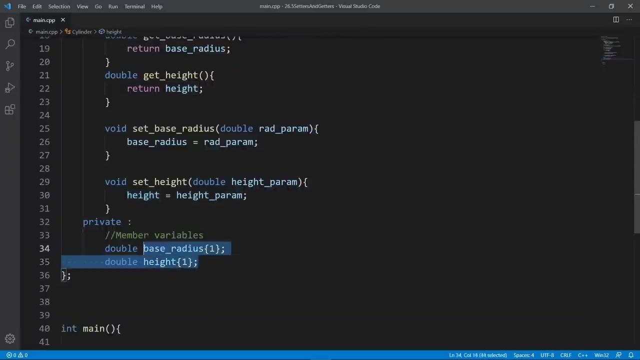 member variable, we're going to say height and we're going to say height param. okay, so this is our thing here now. we have two functions to get stuff from our class and we have two functions to set data to our member variables. here and again, remember that we can't have direct access to these. 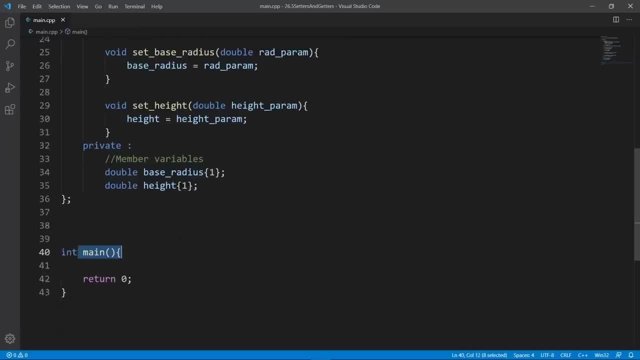 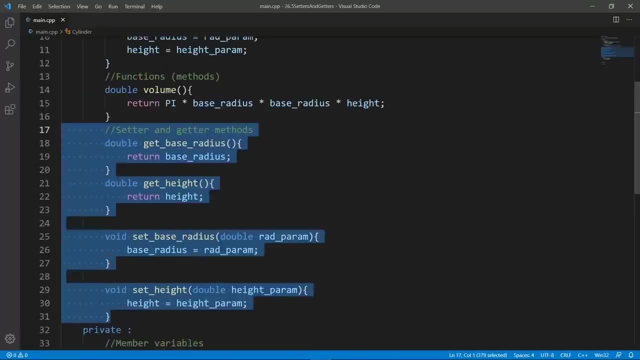 member variables on the outside of the class. and if we want to do that, we're going to be able to do that through our setter and getter functions. now, for these functions- setters and getters- to be accessible from the outside, they need to live in the public section of our class. 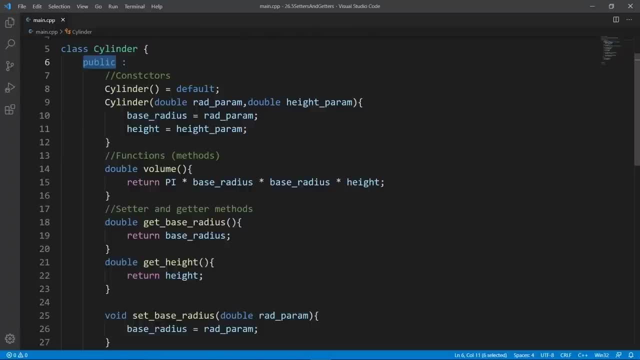 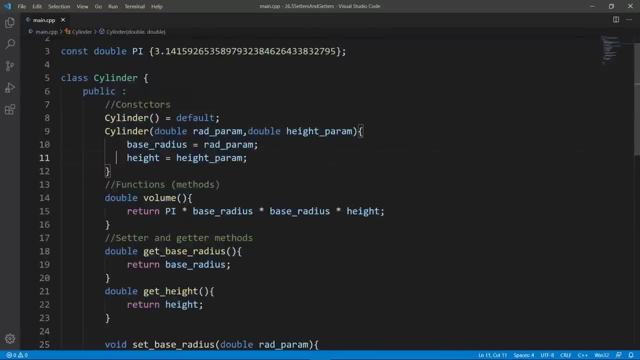 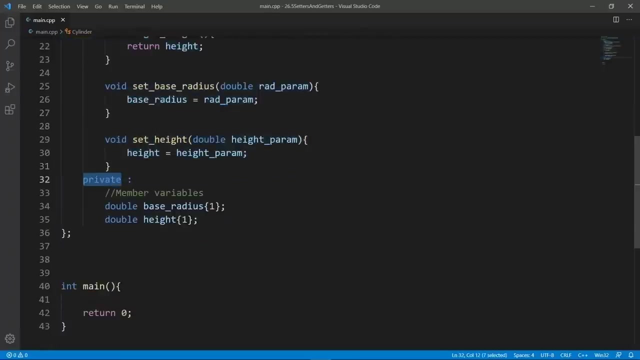 you see, this public keyword here is going to apply to anything after it until we change this to private somewhere. so the public scope is basically going from the constructors here all the way to our set height function, and once we put this private keyword here, everything after that is. 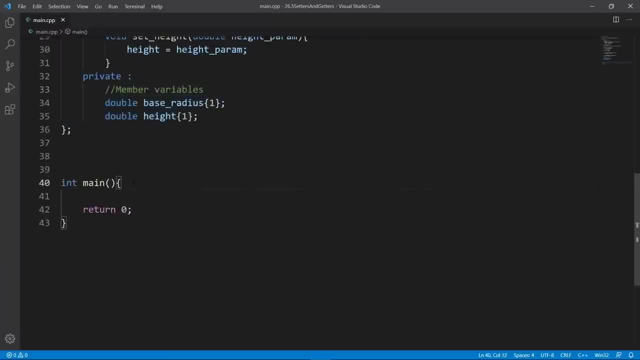 going to be private. this is how these things work, so let's try and use this in main. we're going to set up a cylinder object, cylinder one, and let's put in, for example, two and three- why not? and now, if we want to have access to the base radius, remember if we tried to access that directly. 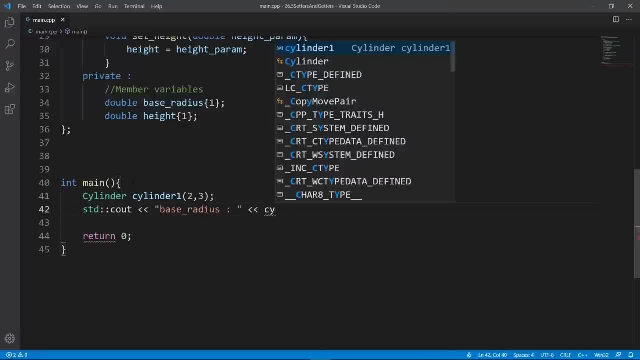 let's say that if we try to do something like cylinder one and say base radius, you're going to see that we're going to have a squiggly line, meaning that there's something wrong with our call here. let's bring up a terminal and see what visual studio code thinks about this. members of 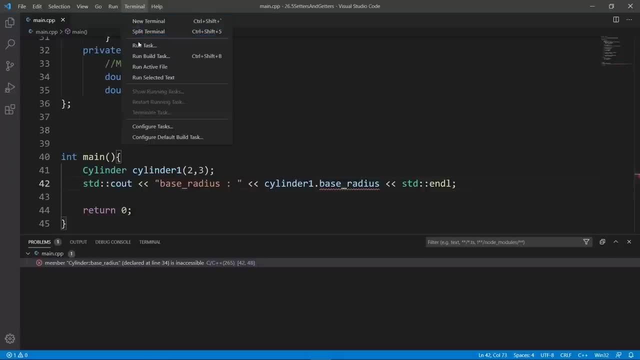 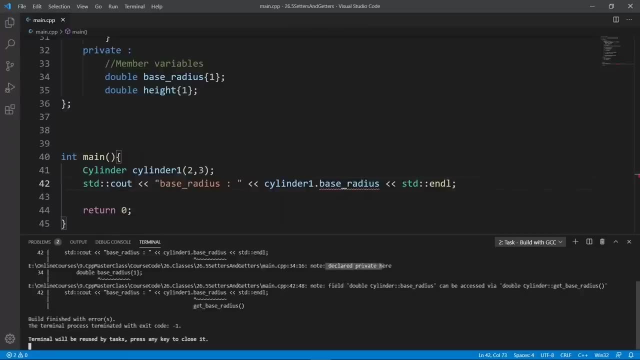 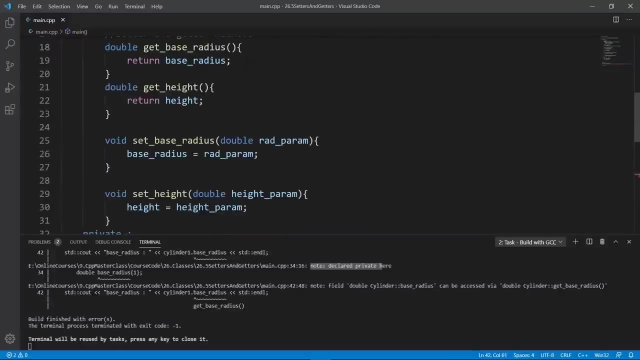 the base radius declared this in accessible here. if we try to build, we're probably going to get a compiler error that says that base radius is private in this scope and that's what we have here declared private here. so we can't access this from the main function here. but now that we have our getter functions we can go through. 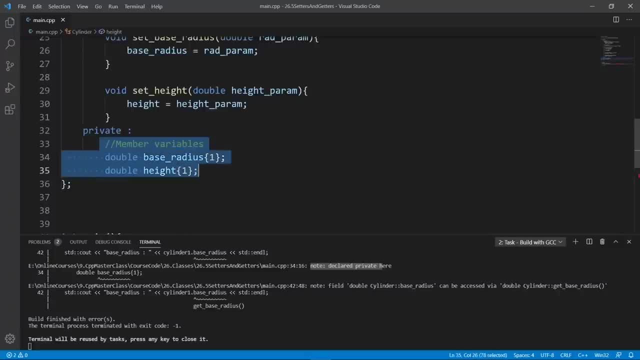 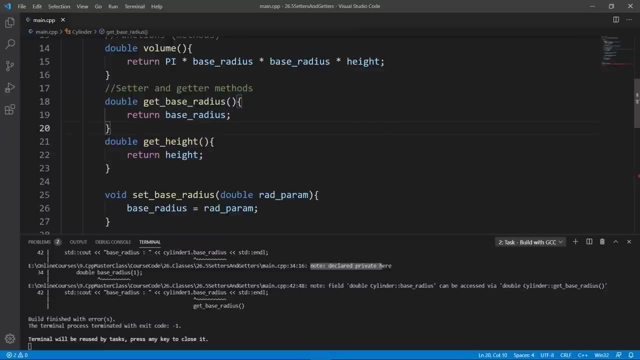 them and have access to private member variables and notice that because we are returning by value here, what return is going to be a copy? you really need to keep an eye for whether what you are manipulating is the original stuff or a copy. so here we're going to be returning by. 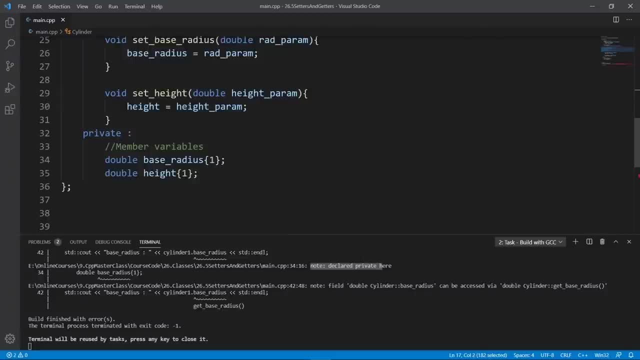 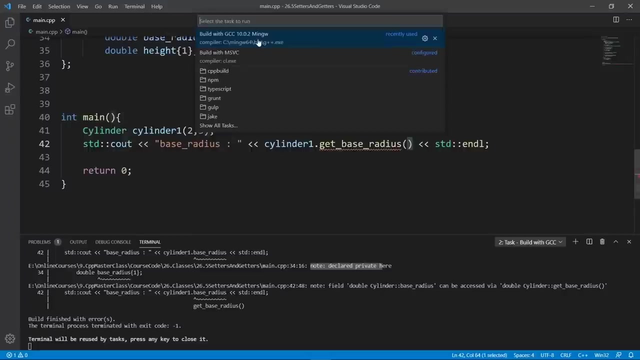 value and we're going to return a copy. but this is still useful in some cases. so here we can use our getter. let's take out this here and say: get base radius. it is a method or a function, so we need to put our function call here and now. if we try to build, let's pass this through gcc and see. 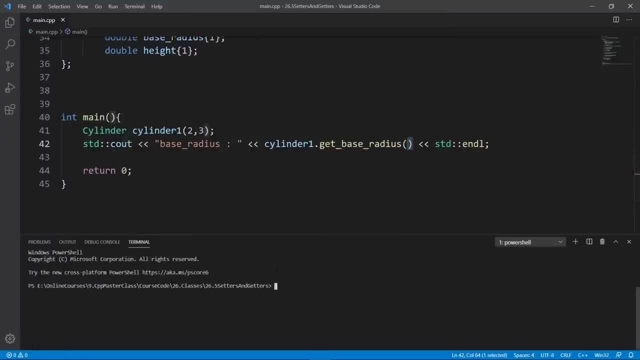 what we get. you see, the build is good. we can run this program. let's clear and run rooster. you're going to see that the base radius is two. now, now that we have this stance, we can actually modify stuff about our cylinder here. let's put in 10 and 10, just to be. 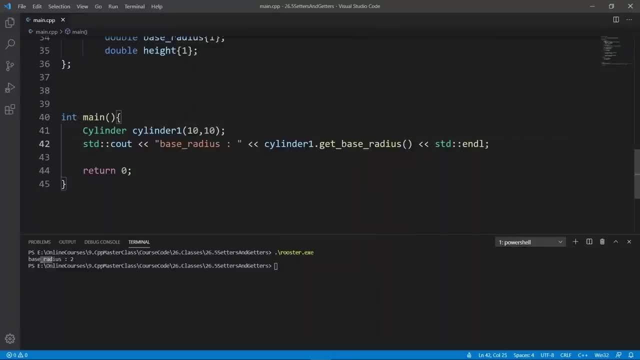 able to follow this easily. and we're going to print the volume. let's say volume and we're going to say volume here we're not going to use the getter. here i'm going to say volume. this is going to print our volume, but we're going to modify our member variables. remember, this is an object. 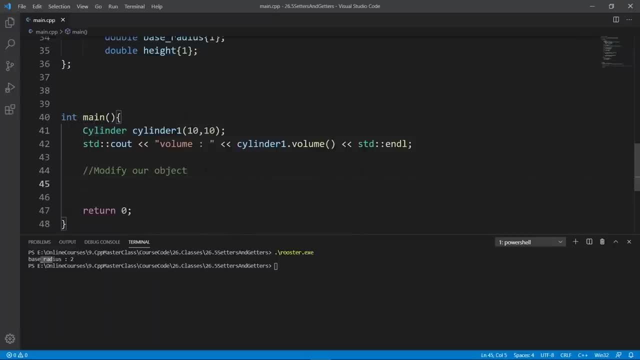 of the getter and we're going to print the getter and we're going to print the getter and we're going to print our cylinder class. so we're going to say cylinder one set base radius. we can do that and we can change this to 100, for example, and we can change the height. that height, we can use this. 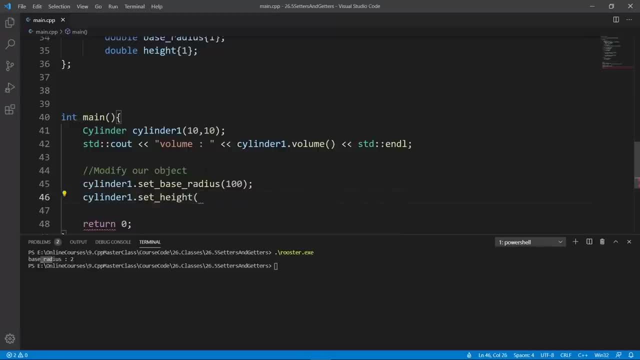 member function because we have it now and we're going to set this to 10. why not now? if we print the volume, you're going to see that the volume has changed because we are going through our public setter and getters methods. so the cylinder is now going to be used to set the getter and getter. 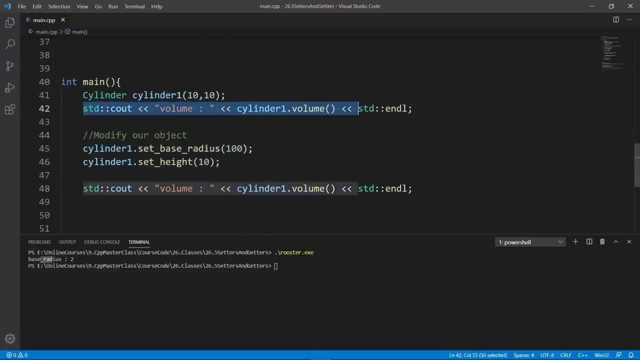 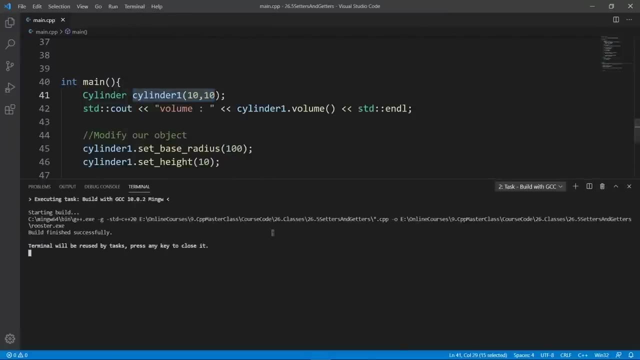 and for the first case here the cylinder is going to be using the data we used in our constructor. here let's build and run this application. the build is good. we can clear and run rooster. now, for the first time, we're going to see that our volume is this number, and for the second time, 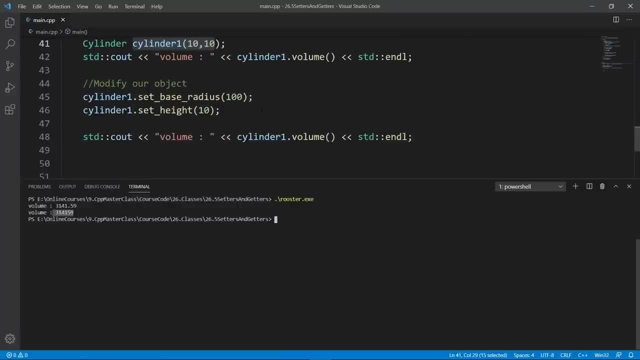 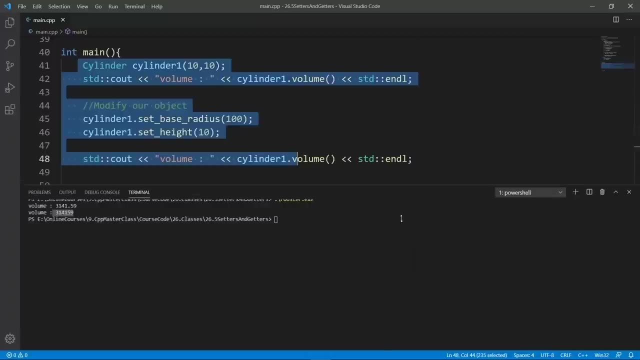 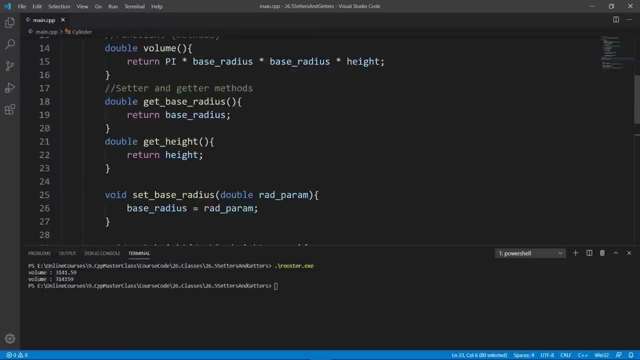 our volume is going to be multiplied by 10 because we changed the base radius to 100, and if you put these numbers then you're going to see that they make sense. we are able to modify our member variables through our setter and getter functions. and again for this setter and getter, 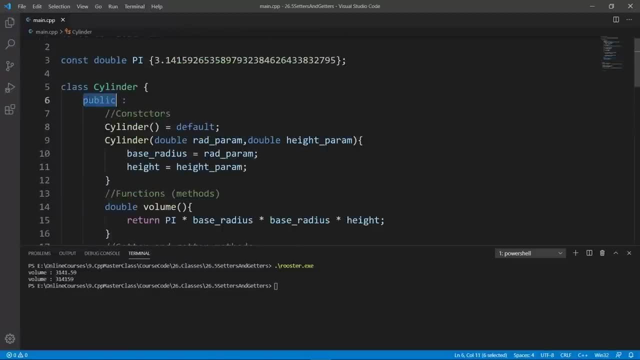 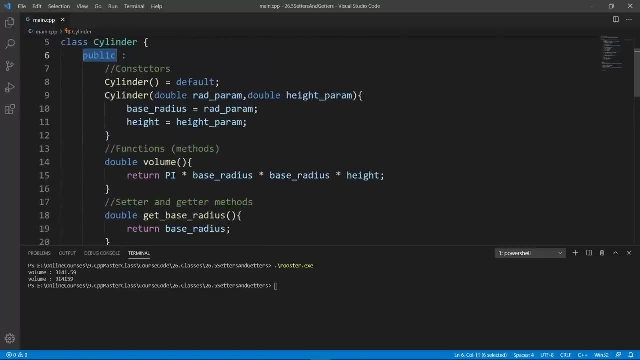 functions to work, they have to be in the public scope of your class, because if you make them private they're not going to be accessible from the outside and you're going to get a compiler error. let's try and do that. we are learning, so we're not afraid to break things a little bit. so 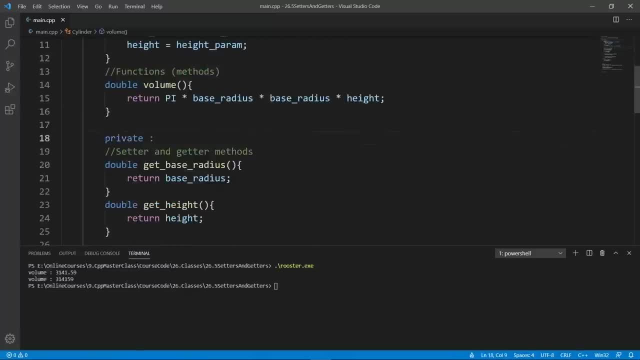 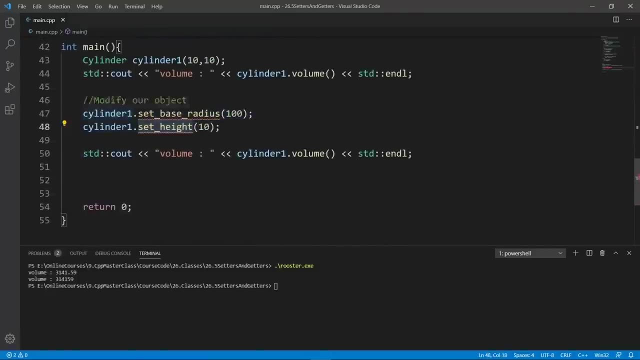 let's make them private. we can do that and bring this a little bit to the left, and at the moment we do that. we should have a few squiggly lines in our main function and we do expect this because they are private now, so we have no business accessing them. 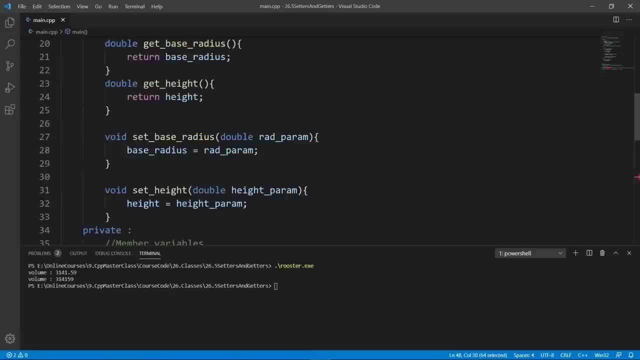 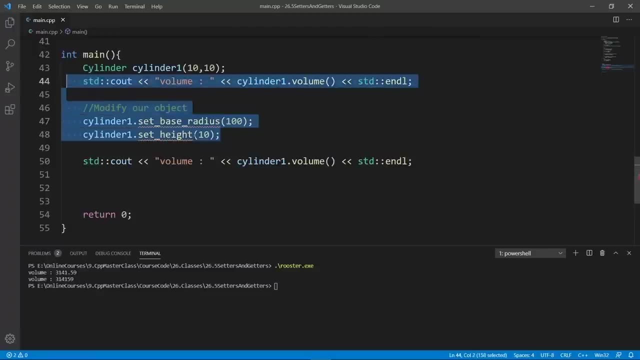 from the main function like this. they are meant to be used from the inside of the class. if they are private, like this, and if you try to use them from the outside, you're going to get a compiler error. let's pass this through gcc to really see the compiler error and we're going to get set. 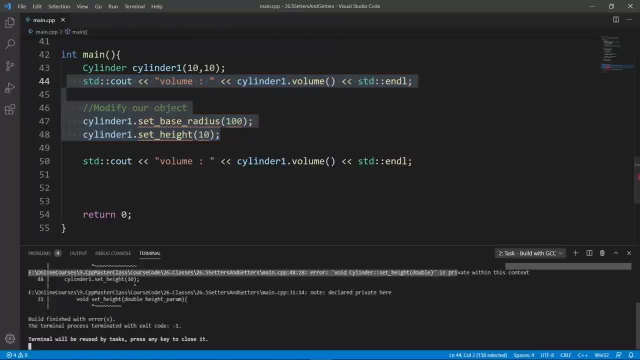 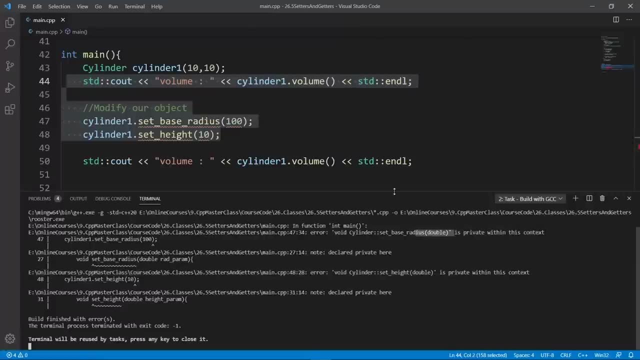 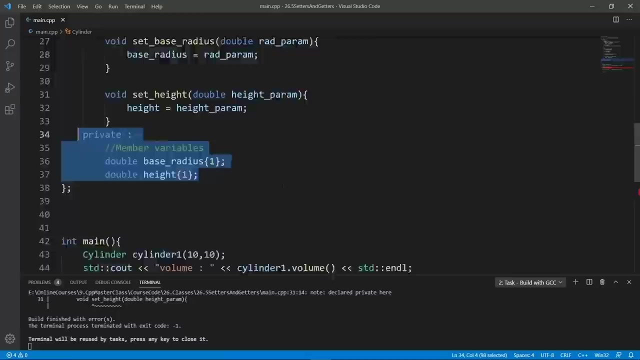 height is private from the context of the main function and if we go up, i think we're going to see the same thing for a set base radius. and that's here. this is really all we set out to do in this lecture: showing you how you can use setters and getters to manipulate your member variables from the outside. 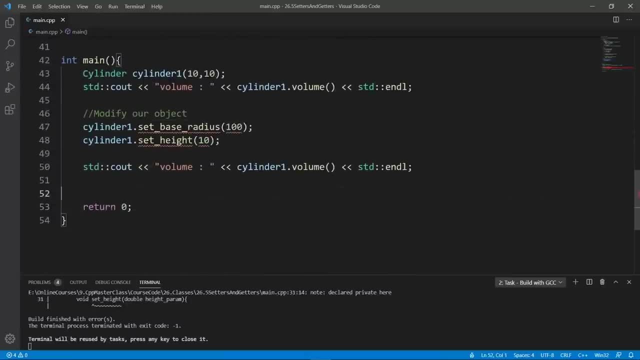 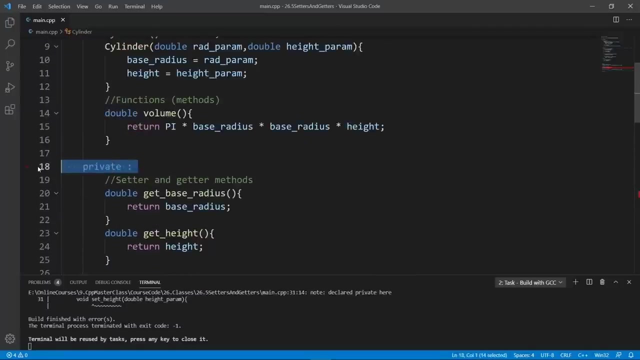 and i hope you found this useful. we are going to stop here in this lecture. in the next one we're going to show you how you can split your class across multiple files. but before i let you go, let's fix this so that we don't have a compiler error here. so we're going to remove this private. 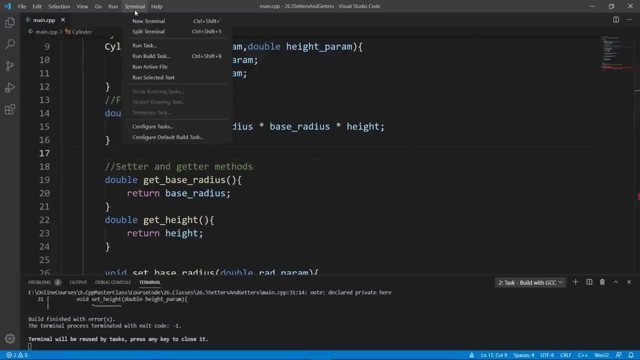 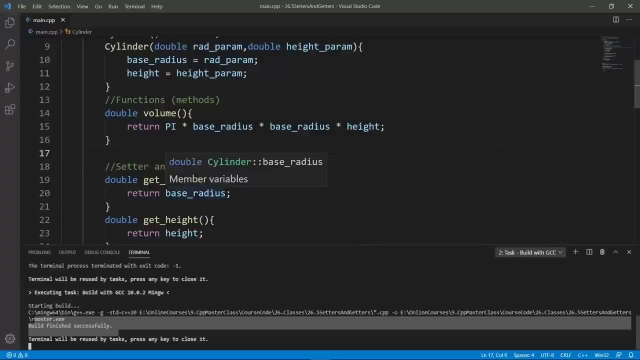 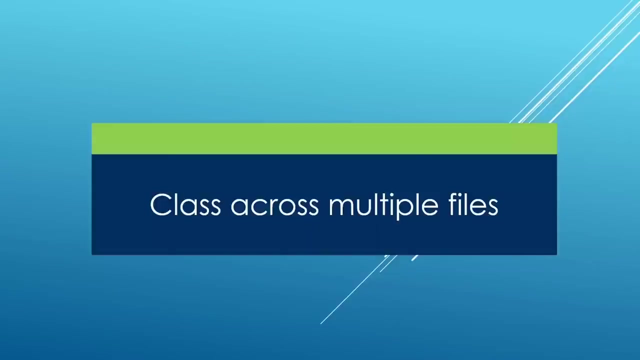 keyword we have put here and we're going to build again. to make sure the build is good, let's use gcc for that. the build is good and i will see you in the next lecture. go ahead and finish up here and meet me there. in this lecture, i am going to show you how we can split our class. 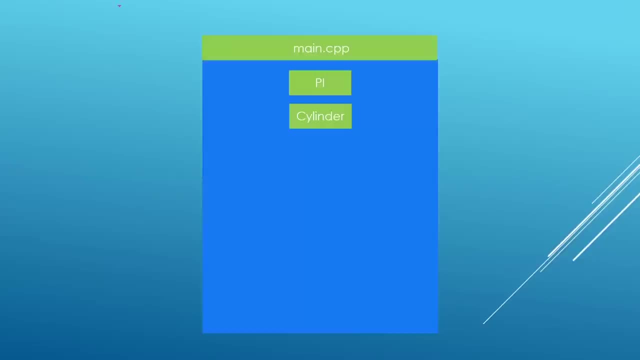 information across multiple files. so far, what we have been doing is really cramping everything in the main function. we had our constant declaration, we had our cylinder class definition and we had our main function to use. these things all cramped into the main cpp file. now we're going to see how we can do things better. the first thing we can do is move our constant in. 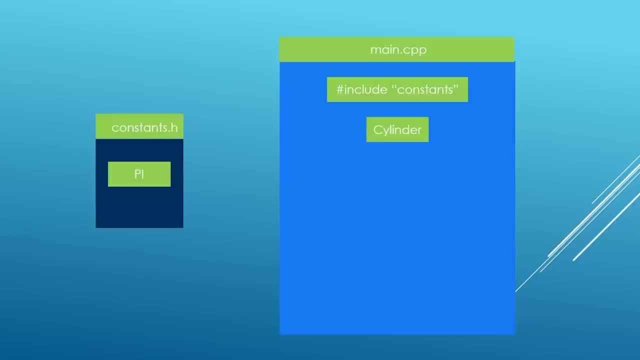 another file because, if you think about it, users of your class in the main function don't care about this constant pi, because it really is an implementation detail that should leave somewhere else or even inside the cylinder class. but we're going to put this in a separate file because that's going to give us room to put as a 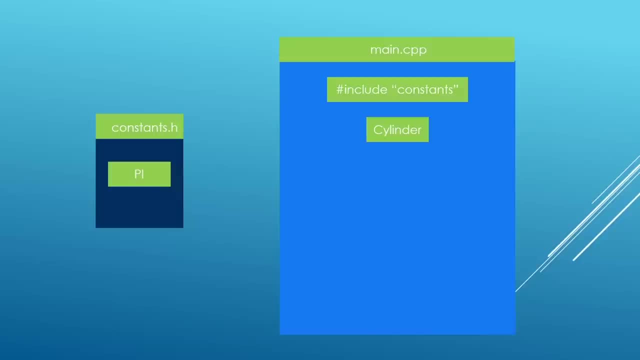 constants if we need to do that. so if we split things up like this, when we want to use the pi variable, we will need to include the constants file, because that's going to give us access to it, but we don't have to maintain it in the main function. so this is a little better, but another. 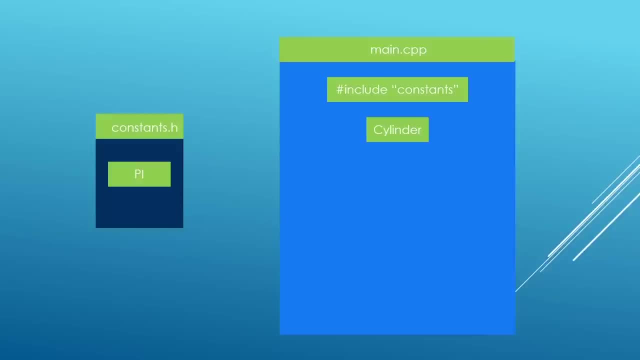 thing we can do is move the cylinder in another separate file and do something like this. so now you see that our cpp file is now in the main function, so we're going to put this in a separate file because, if you think about it, users of your class in the main function don't care about this. 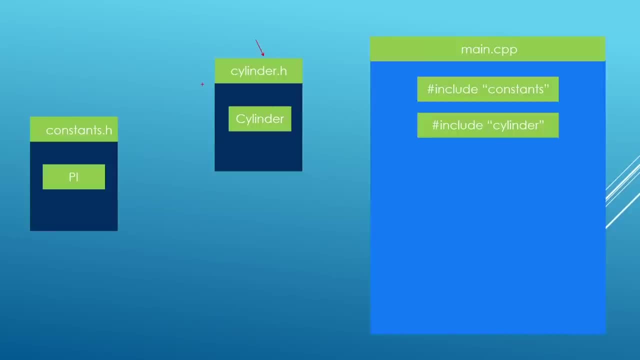 cylinder declaration and definition has moved in a file called cylinder dot h and we have our constant pi living in another file called constants dot h and if we want to use our cylinder class like we have been using it all along, we will need to include the header that brings it in and this: 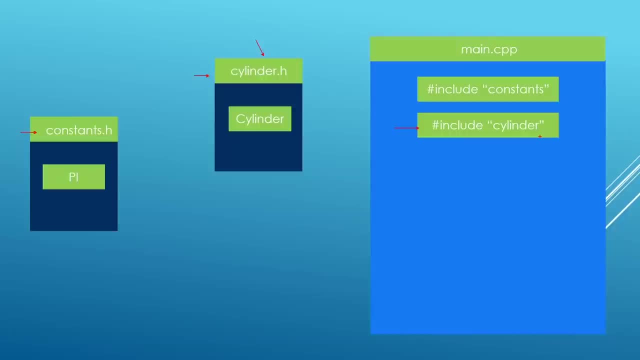 is how we're going to do it and we will be able to use it in the main function if we set things up like this. but we can go even further. we can split the cylinder in another file and do something like this. so we're going to split our class declaration and definition in two separate files. what we're 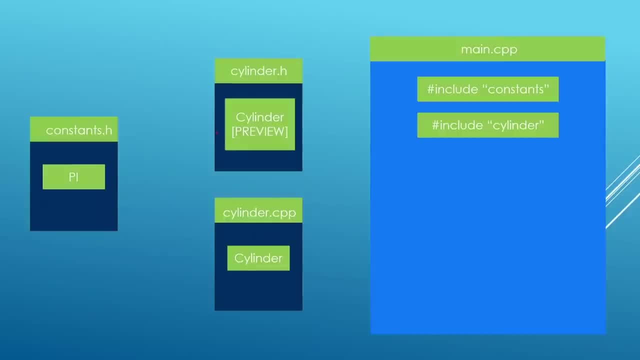 going to have in the header is going to be really a preview of the class and in the cpp file, which is going to be called cylinder dot cpp, we're going to have the implementation details of our class and again, this is going to make things a little easier to manage, because it's really not good to 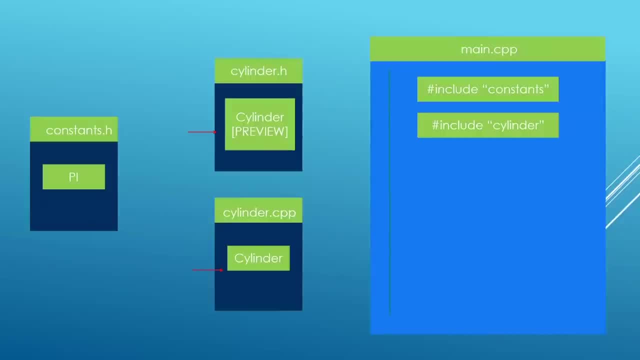 have everything cropped into your main cpp file. it should really have high level details about how your application works, and all the low level details should be split into different files. this is good design. now that you have an idea about this, let's head over to visual studio code. 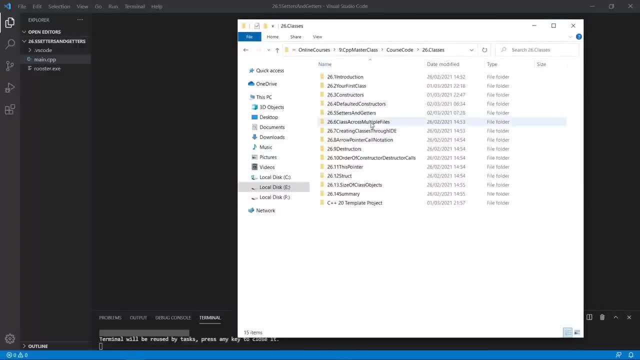 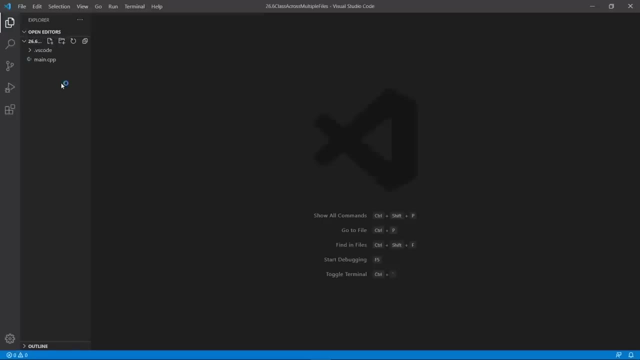 and show you how you can do this. okay, here we are in our working folder. the current project is class across multiple files. we're going to grab our template files and put them in place, and we're going to open this in visual studio code so that we can really play with us. this is going to open. 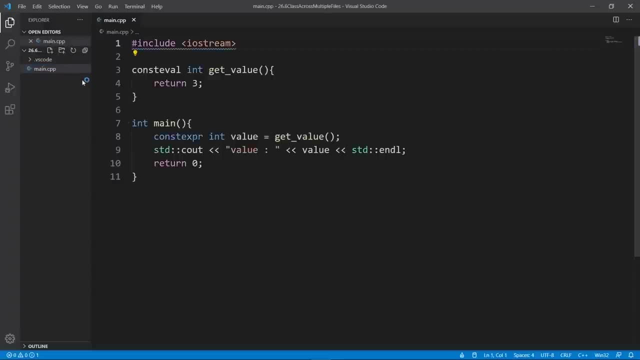 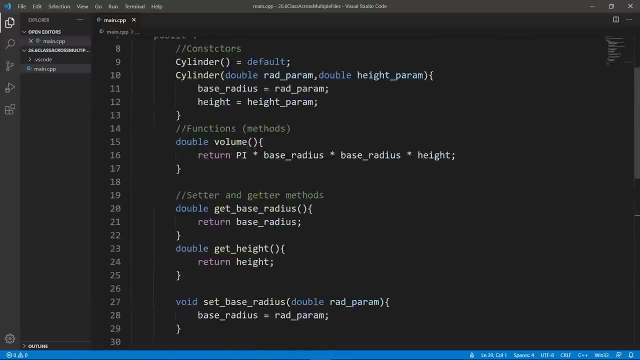 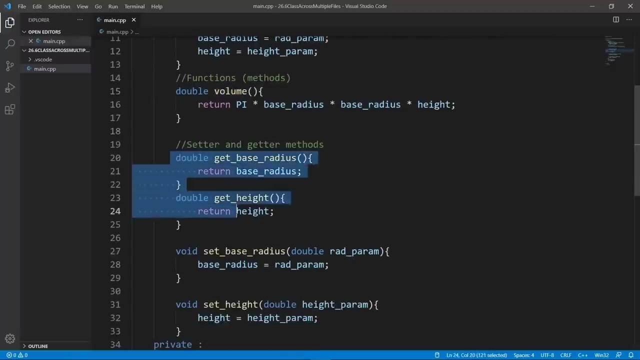 our folder we can open the main cpp file. we are going to clean it up a little bit and we are going to grab our class definition and put that on top here. so this is our cylinder class. we have the constructors, we have the functions, the volume function here- and we have our setters and getters. 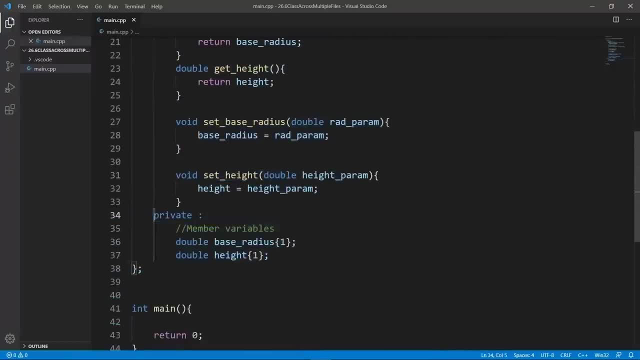 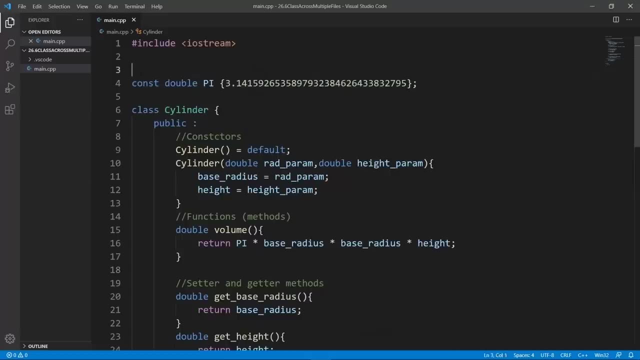 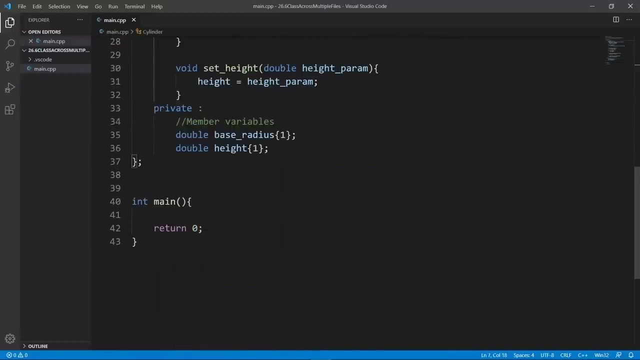 inside down, we have our member variables, which happen to be private to this class. here. now, what we want to do is to organize our code better, and the first thing we need to do is to move this constant from the main file here, because it's really not that useful at this point. 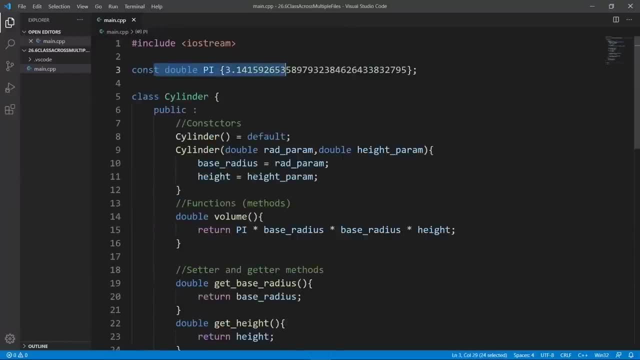 here. users of your classes won't really care about what pi is, because it is an implementation detail to the cylinder class, because we are using that to compute our volume. so this constant really has no business being in the main file. we're going to move this in a separate file. we're going to set up 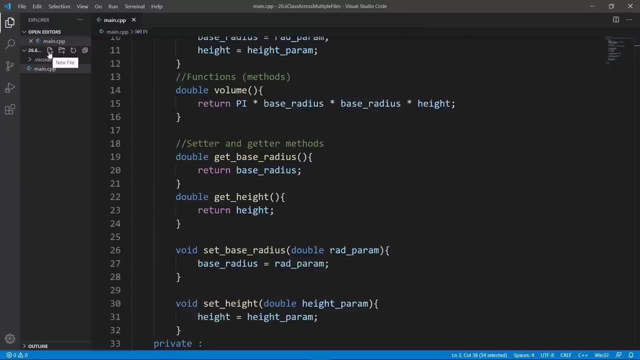 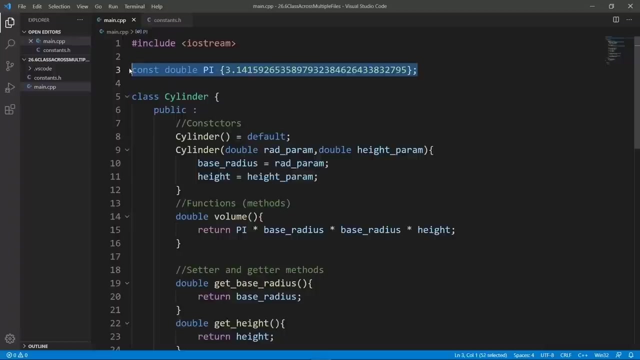 a new file. we're going to come to the left here. click on the plus icon here that says new file. we're going to say constants and we're going to call this constants- that h, because it's going to be a header file and we can just come from the main cpp file. we're going to copy this. 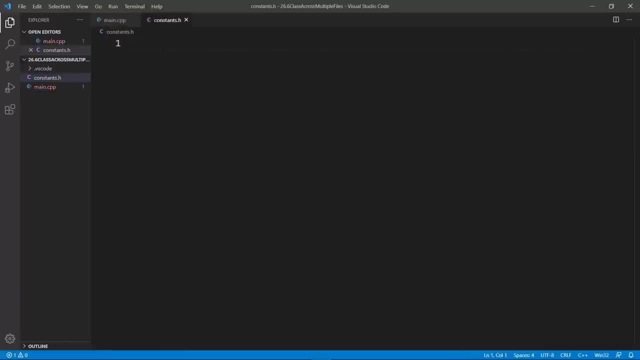 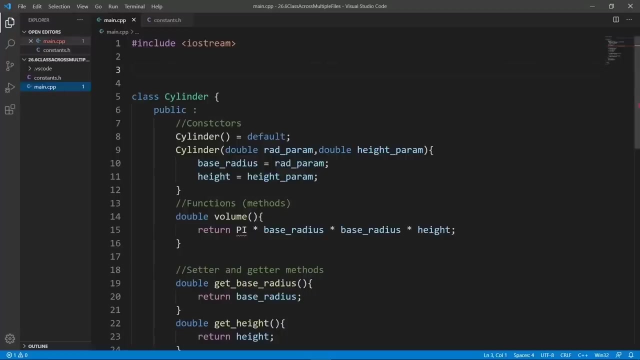 we're going to cut this actually and we're going to put this in our separate file, which is constants that h. after we do this, we're going to come in our main cpp file and we're going to include that header file. so let's do that. we're going to include constants that. 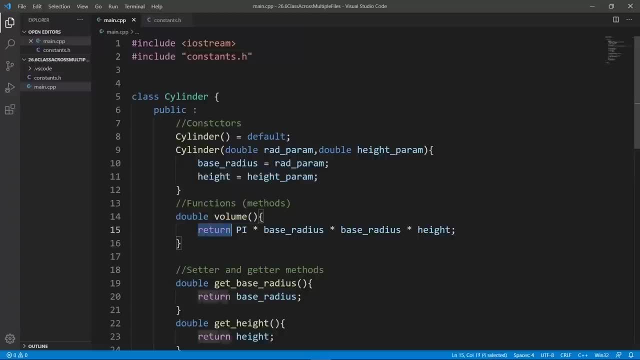 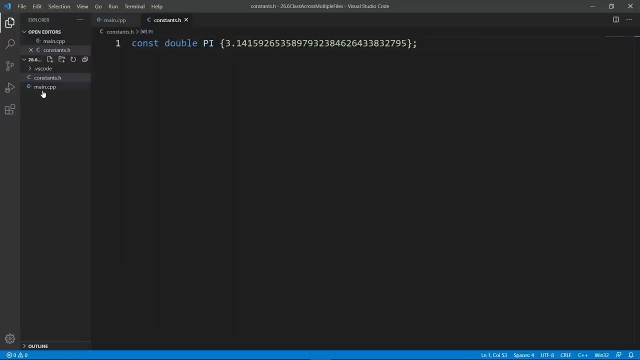 h, and the moment we do that, you're going to see. now visual studio code knows where this constant is, but we don't have to deal with that directly here. another benefit of doing things like this is that we can go in this header file and declare thousands of other constants and we can have 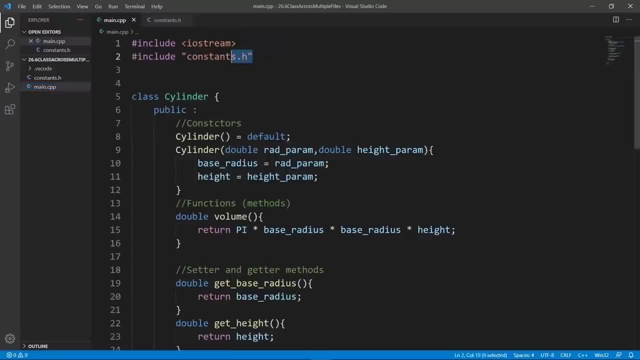 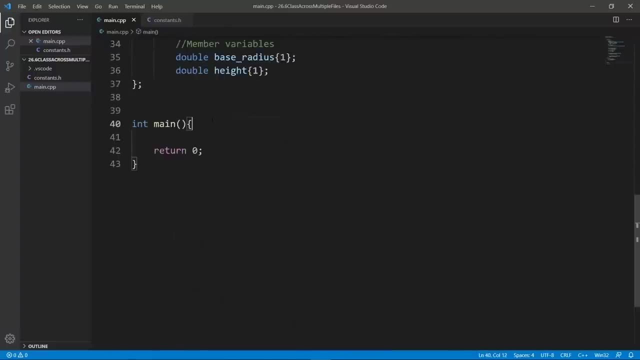 access to them in the main function by just using this single line that includes our file here. so this is good design. if we build our application, you're going to see that it is going to work. let's dead nos to this. actually we'll. let's wait for a second. i'll just show you something i'll wait for. 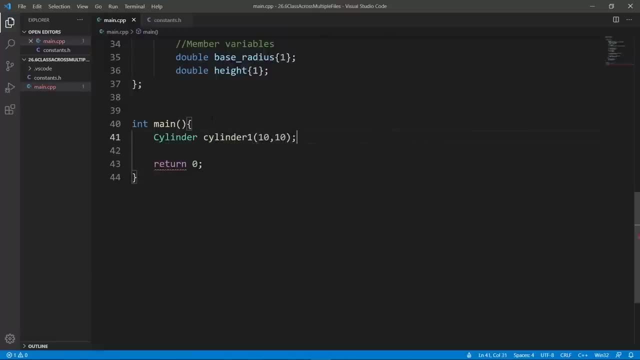 so let's okay, and i see that i need to go back to my cpp file. guys, again, let's get going. so let's go ahead and we're going to add a client. so in this case, we choose a client, so we're going to add interior. material here. so for the time being, i'm going to make a client called a loop, and what i get out is this: right now we're going to be setting up a今 case. we're going to say cylinder object, we're going to say cilinder one, and we're going to put 10 and 10 n as our parameters and we're going to print the volume of 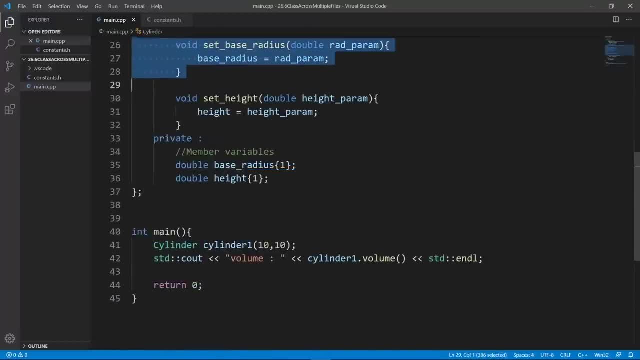 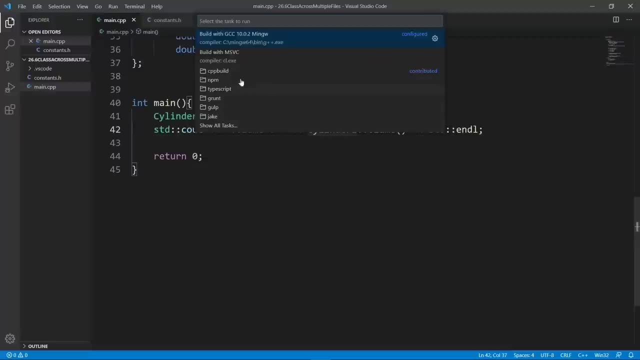 that's going to be the member functions of a class, so don't be confused by this right here. if we build and run this application, it should be working right, because we have everything we need for it to work. let's see if the build was good. the build was good. we can bring up a terminal. 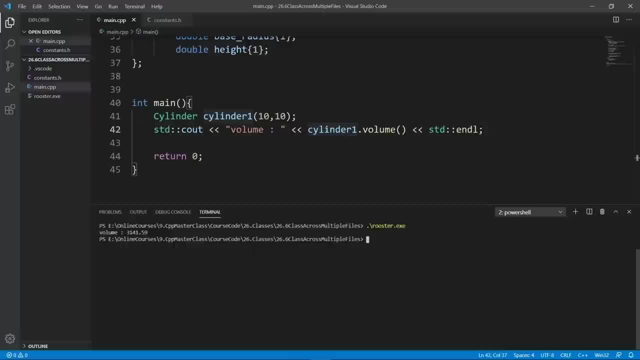 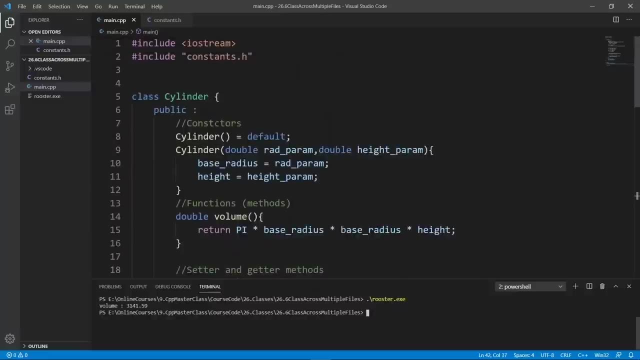 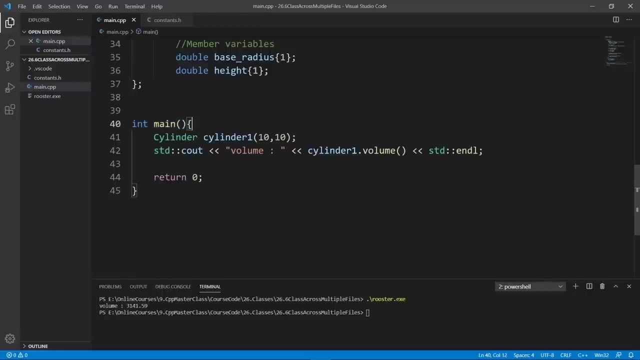 and actually run this. let's clear and run rooster. this is going to print our volume, so the code is working right. the second thing we want to do is to move this class all together in another file, because we don't really want to see it here in the main function. what we really want is to use stuff. 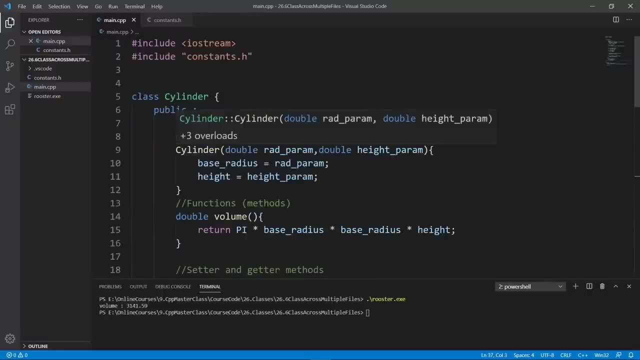 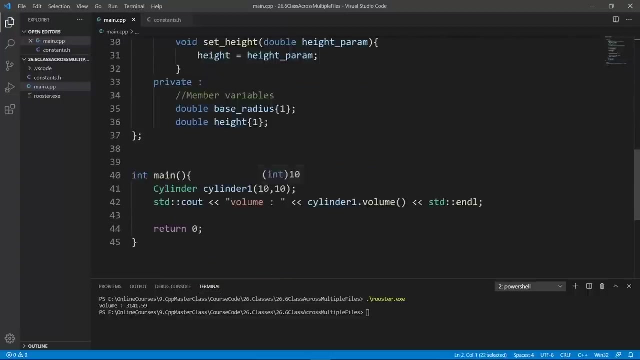 and we don't care about how those things are set up. in the same logic we used when we used std strength, we didn't really care about how std strength is put together. all we really wanted was to include the class that brings it in and use it in our code we're going to be setting up. 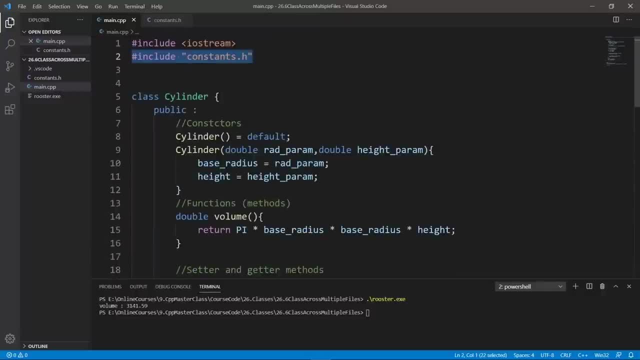 the same behavior for our cylinder class here, and it is going to be instructions and it is going to show us that this is the above and่ to be living in its own separate file. so let's set up another header file. we're going to call this cylinder dot h and we're going to grab our class definition all together. so we're going to 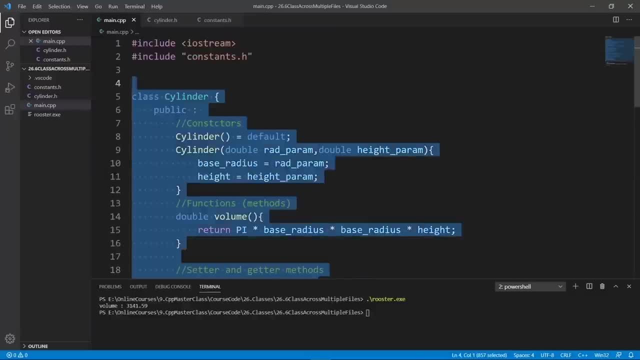 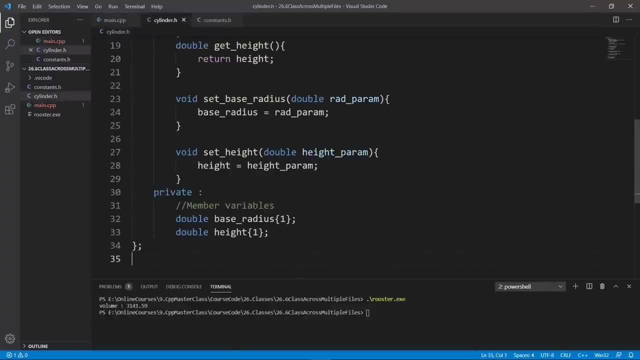 go from the bottom here and select everything that includes our class. we're going to cut this out. we're going to go in our cylinder header and we're going to paste this in there and we're going to come back to our main file and include our cylinder class. so let's do that. we're going to. 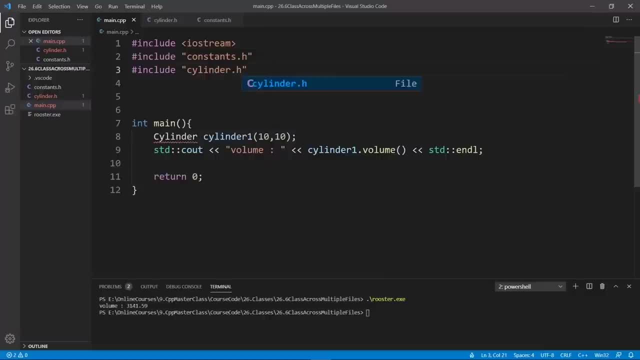 include, and we're going to say cylinder dot h, and this is going to make things work. remember, the preprocessor is going to put these things in. the preprocessor is basically going to go in constants, it's going to take whatever is inside and then it's going to paste that here and it's going to 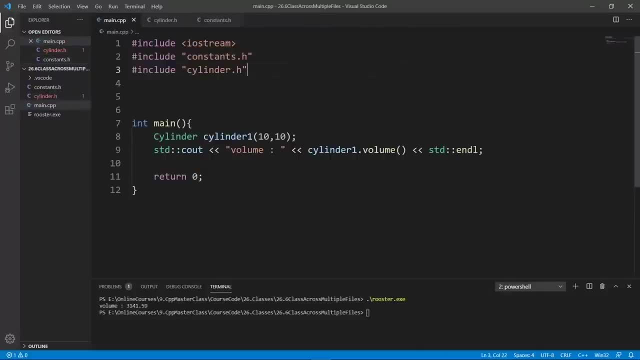 take everything inside our cylinder class and it's going to paste that here. so it's basically going to be like we are declaring these things in the main function, but our code is going to be better organized now. if we try to build this program, it is going to world exactly like it did, because we have all 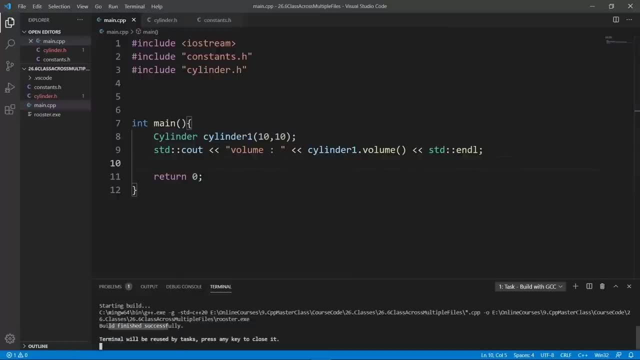 the information for it to world. let's world. world is finished successfully, so the world is good and we can run this program and it's going to do what it was doing all along. we can clear and run rooster. don't worry about visual studio code here. i don't know what the problem is with that. it's. 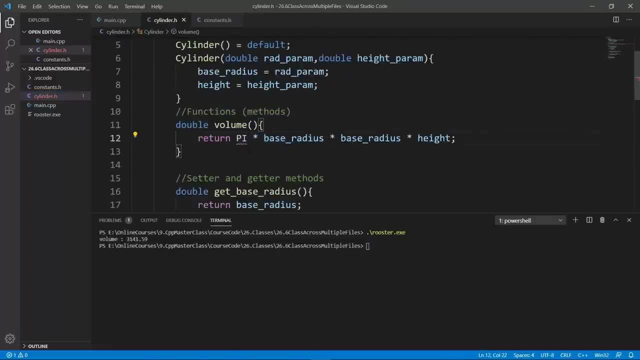 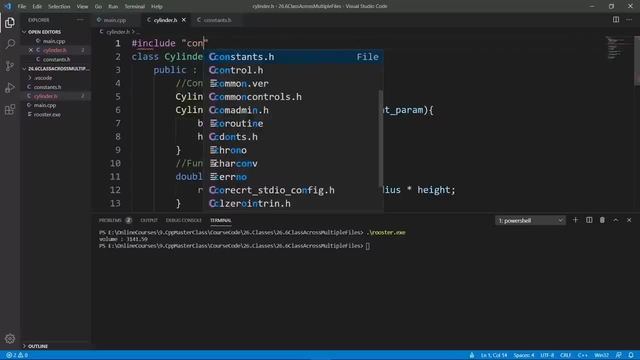 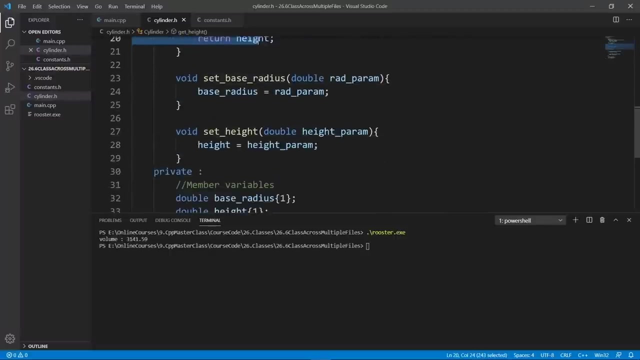 just having. ah, it's having a problem with the pi constant here because it's not included in here. so what we can do is say include and include our constants header, and if we do this the problem here is going to go away. but we're going to have a problem if we're trying to run this program now. 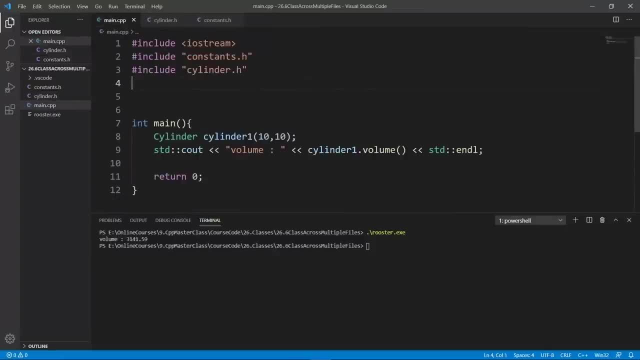 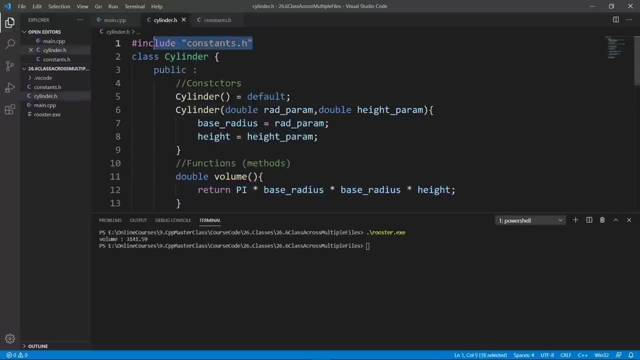 because- try to think about it- in the main function we are including the constants header and in the header of cylinder we are also including this little guy here. so if the processor comes, it's going to include this and it's going to have this little guy inside our main function and the cylinder is also going to include this. because 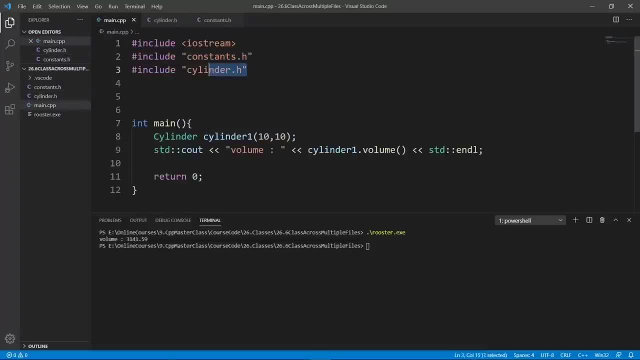 it's including this header. so when the preprocessor is done, we're going to have our constant here declared twice and if we try to build this program, you can expect bad things to happen, because it's really not good to have the same thing defined more than once in your entire program. 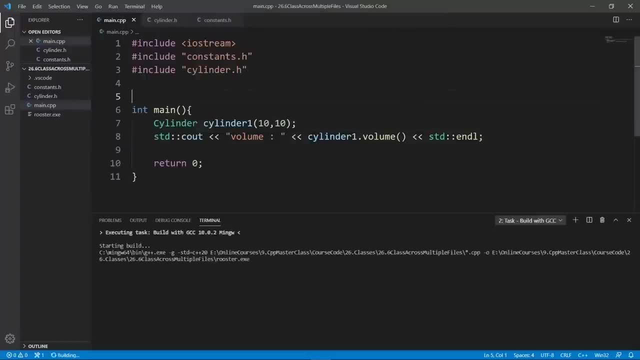 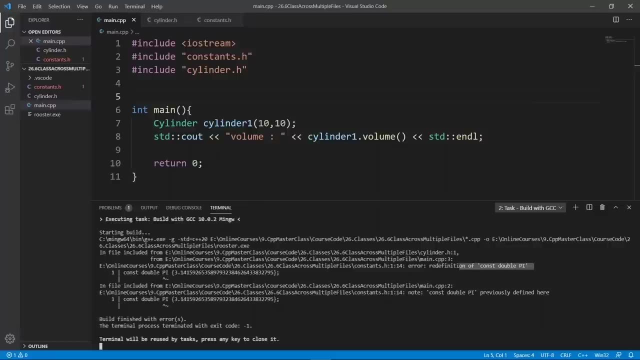 and let's try and build and show you this. hopefully we're going to get a compiler error and it's going to blow up in our face. it's going to say: error: redefinition of const double pi. so what is going on here? we are including this thing twice, once here and at the second time. 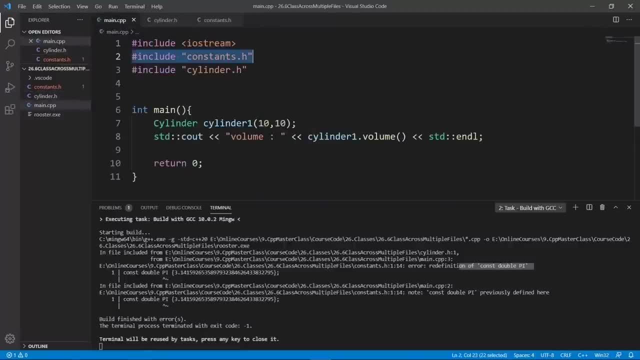 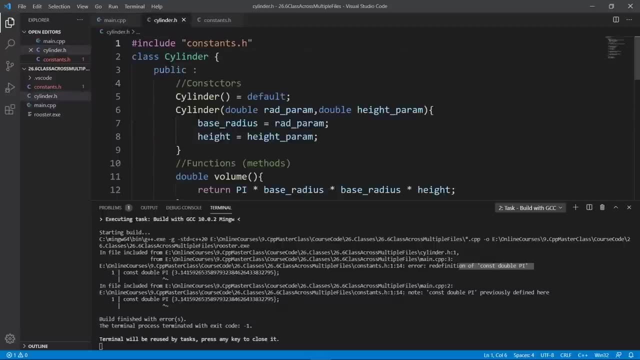 it's coming in directly from the cylinder class, because we are including that in this location here, and what the preprocessor is basically going to do? it's going to copy the entire file here and it's going to paste that in the place of cylinder dot h here. 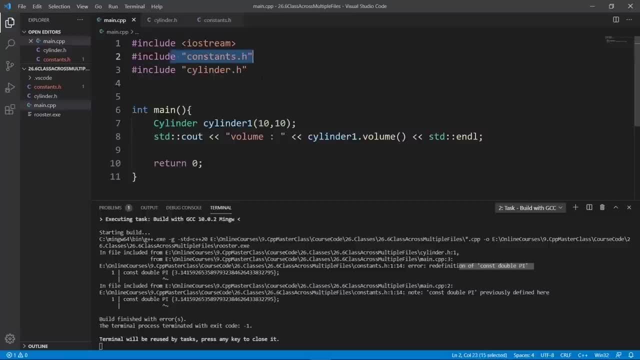 and it's going to paste that in the place of cylinder dot h here, and it's going to paste that. and this constants header is basically going to be included twice, so it's going to be redefined here. that's the problem we have. one way we have to solve this in c++ is by using include guards. 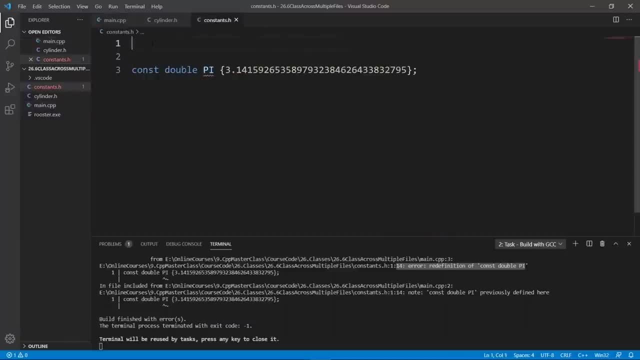 and the way we do that we come in our constants header and we say pound, if and def. this is a way to say if something is not defined yet, and let's say cylinder underscore h, and we're going to say define cylinder underscore h and we're going to come down to the end and say and f. this is a way we have to tell. 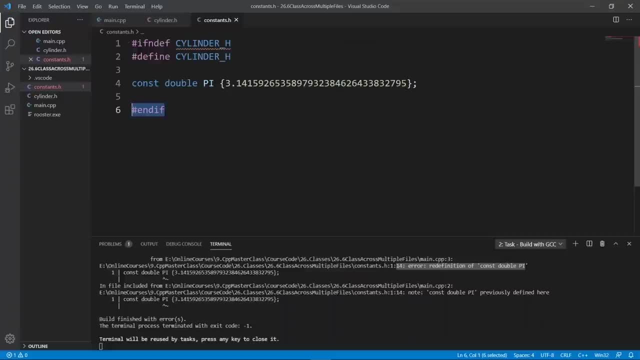 the preprocessor to only do something or include the code we have within these things if the condition on top here is satisfied. so for example, the code inside here is going to be put in our c++ source file if the cylinder name here is not defined in the eyes of the 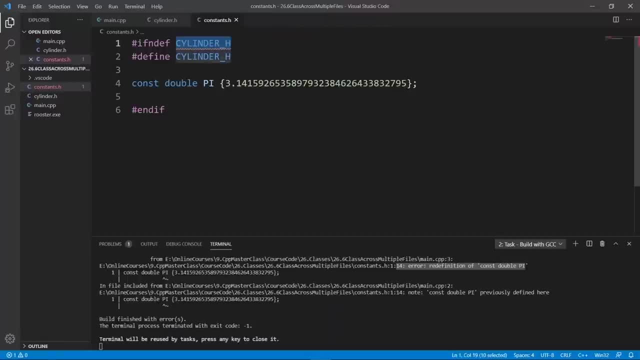 processor. so it's going to say: if cylinder underscore h is not defined, i am going to define that and i am going to put this code here. but if it's already defined, it's going to skip all these things and it's not going to include this. okay, so this is the logic here. and notice, this is really. 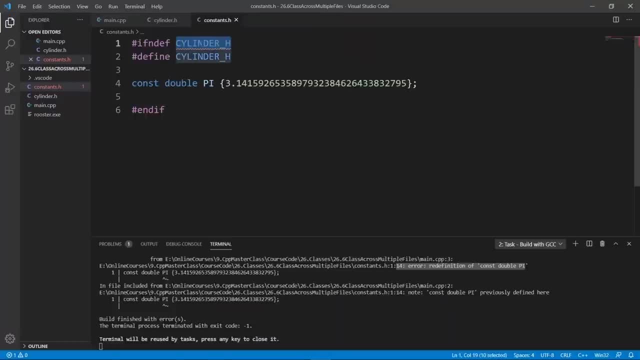 not a cylinder file. so we're going to change this to constants, underscore h. let's say that and let's do the same here, and this is going to do our thing, and we're going to go in our cylinder header and do the same thing, and we're going to go in our cylinder header and do the same thing and we're going to. 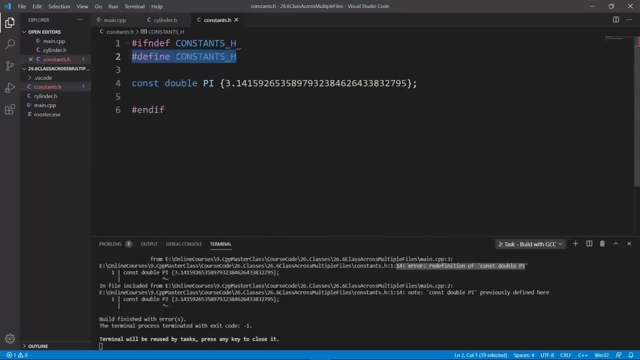 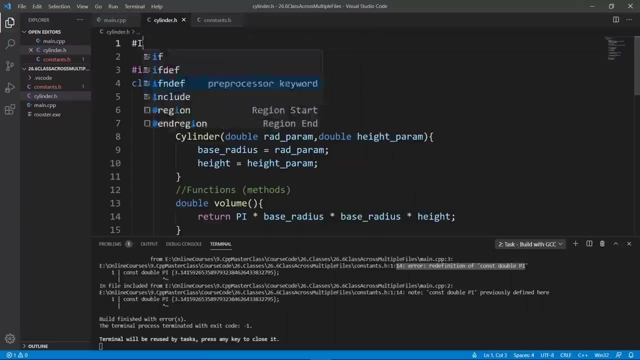 do the same thing and put in our include guard. it is basically a guard that is going to guard against something being included more than once. so let's do that in our cylinder header. so we're going to wrap this inside our include guards. we're going to say if and def. you see visual studio code. 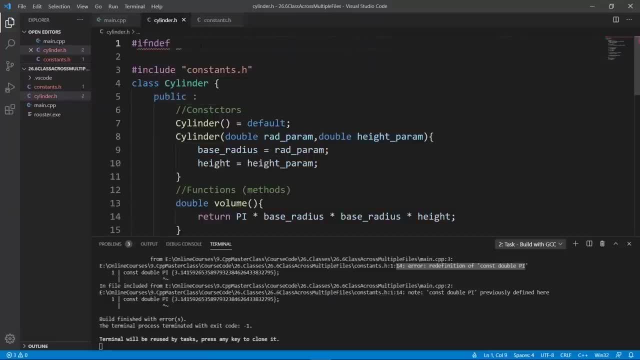 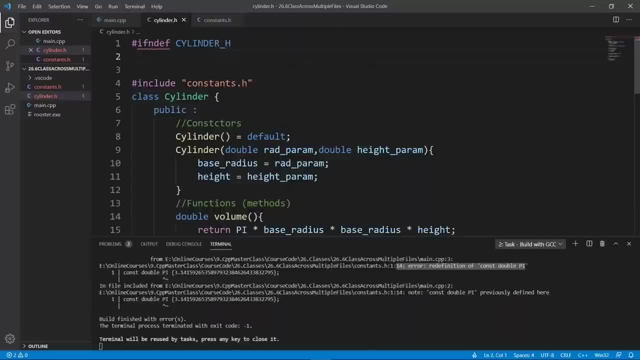 is really helping out here and we're going to put in the name we're going to use for this: this is a cylinder class, so i think it makes sense to call this cylinder, underscore h, and we're going to do the same thing here: define cylinder, and we're going to end f at the end of the. 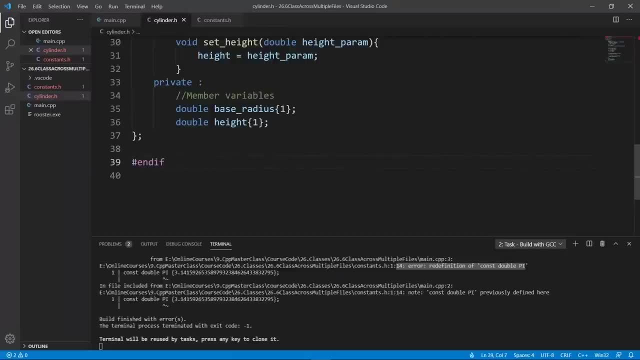 file here. so we're going to say and, f and again. this is the syntax of the preprocessor. i don't want to get too much into this because we will learn about this later in the course, but we can now use this to guard against something being included more than once and if we're trying to 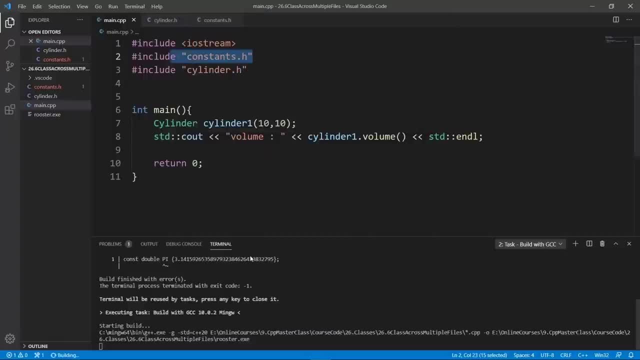 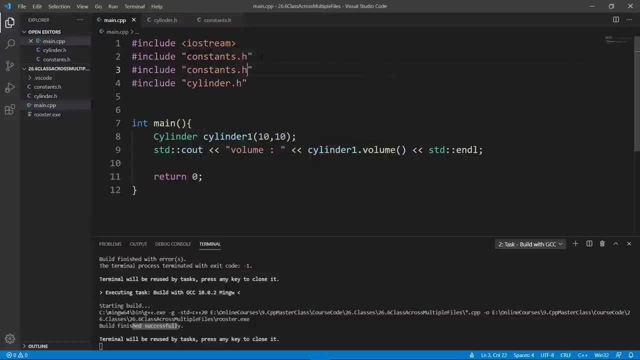 build the program now. hopefully it's going to world. let's use gcc and now you see that the world is good, even if we are including the constants header multiple times in the main file here, we can even go down and do that like a thousand times. so let's do that and you're going. 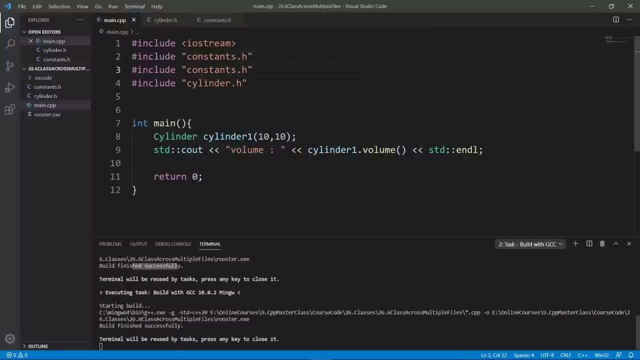 to see that if we're trying to compile, it is going to world fine, because now we have a guard guarding against including this thing more than once. the preprocessor is basically going to come in here and say: if the constants name is not defined, i'm going to define it and i'm going to 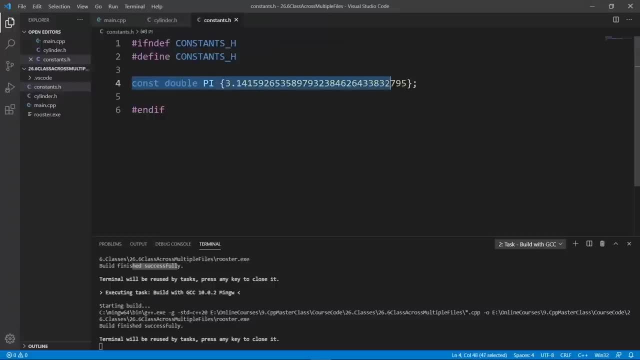 define that name and i am going to put the code here in the source file that includes me, if it happens to be already defined. this condition here is going to fail. it's not going to do any more than in this file. the preprocessor is basically going to give up on this file here. this is what. 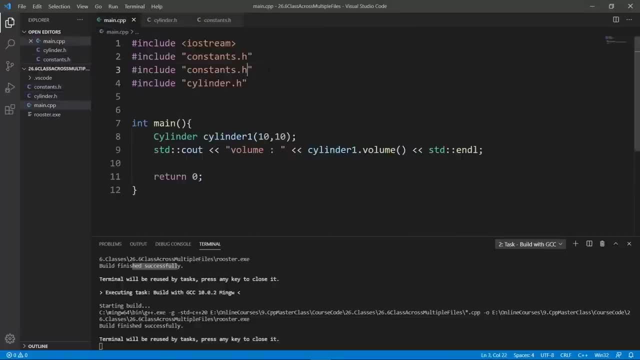 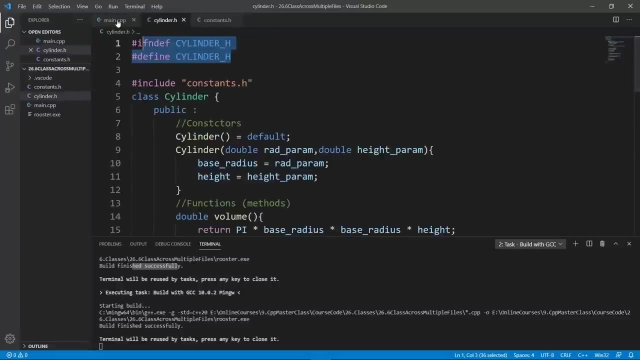 i want you to know. so now we should be able to split our code into multiple files. and now that i think about it, we don't really need to include the constants header here, because it's going to be broadened by the cylinder class, but it was a good opportunity to teach you about the include guards here, now that 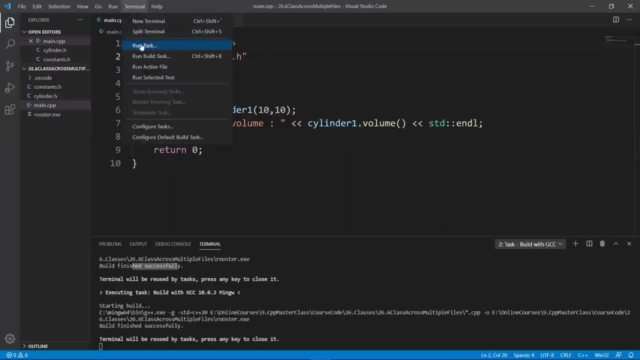 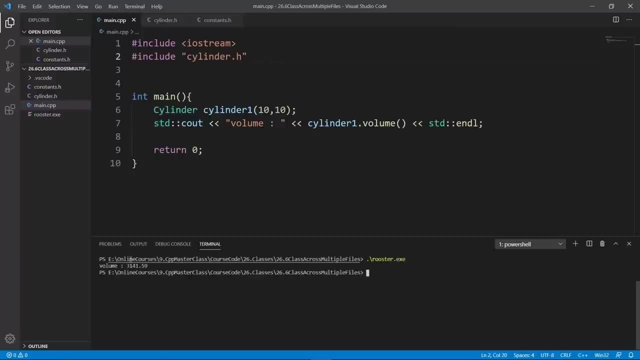 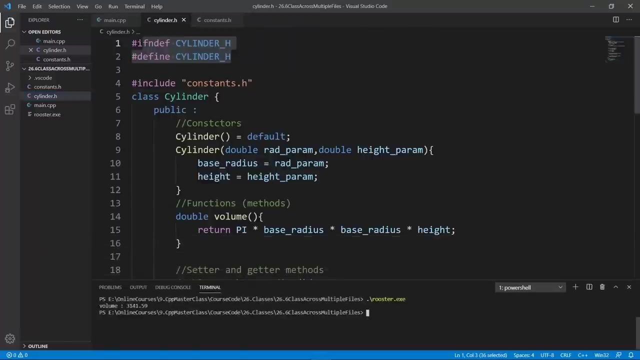 you know this. we're going to remove this and we're going to build and show you that this is going to work anyway. so weld is good, we can run our program clear and run rooster. this is going to work. the last thing i want to show you is that we can go even further and split our class into two separate. 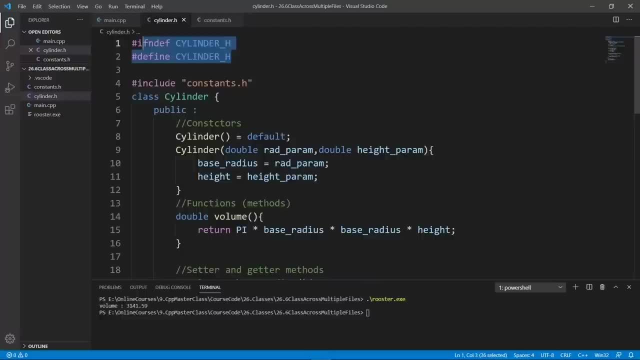 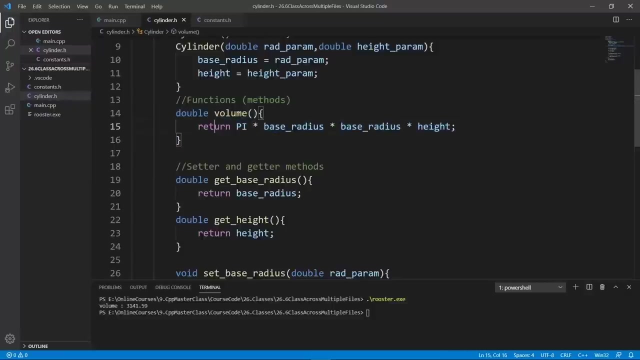 files, because people who come to the header file are usually interested in your class definition and they're going to be interested in your class definition and they're going to be interested in your implementation details. for example, they want to see that you have a volume function and they want to know that they can call that function, but they don't really want to know. 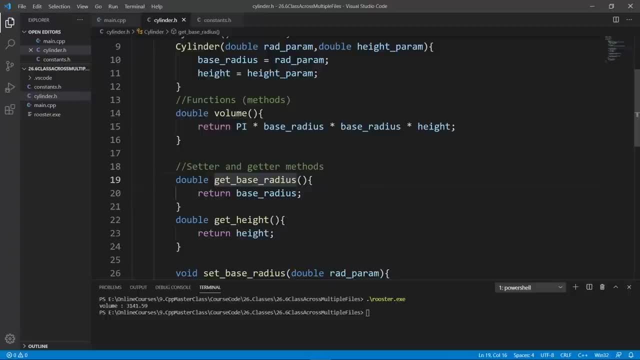 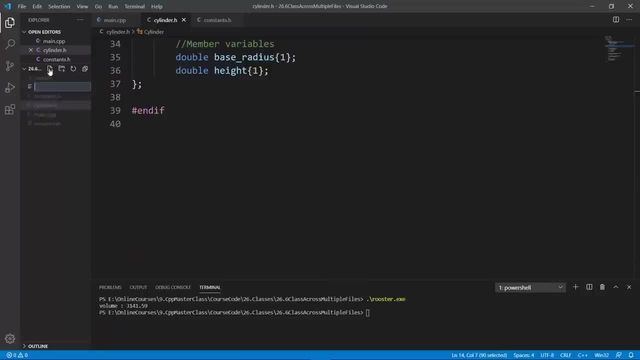 how you compute your volume, and we can really make things simple for them and hide the implementation details in a separate cpp file. so let's do that. we're going to set up a new cpp file, we're going to call this cylinder that's cpp, and we're going to 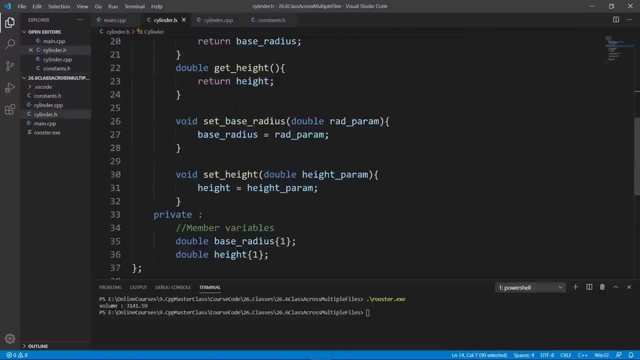 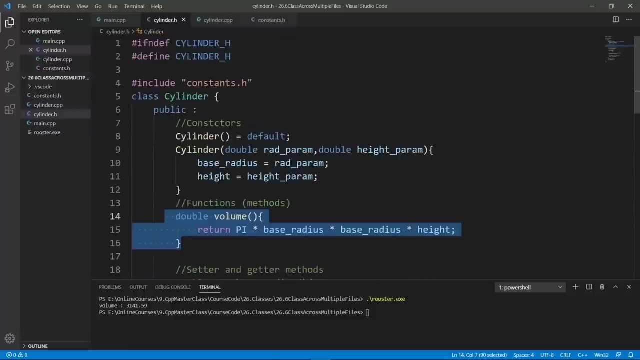 move the implementations of our functions in the cpp file, and i am doing this just to show you that it is possible in practice. you're going to have to decide for yourself what you want to keep in the header file and what you want to keep in the cpp file. so the cylinder default constructor here. 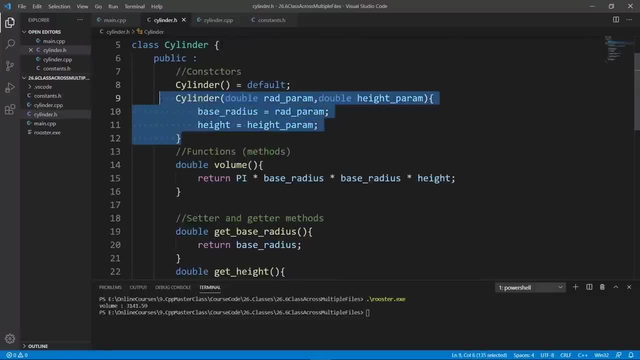 is going to stay this way, but we can move the other constructor here in the cpp file and the way we do that. we're going to just grab this and i am going to change this line by line so that you can see this and in the cpp file, the first thing we want to do. 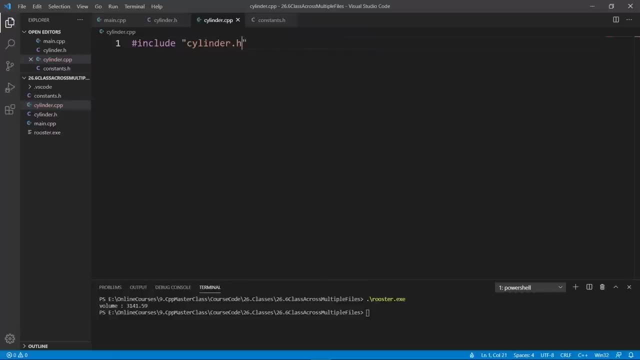 is to include the cylinder header, because the implementations here are going to be using this and we're going to put in our constructor and modify it to be fit for living in a cpp file. so let's come here and do that the way we tell this that this is really an 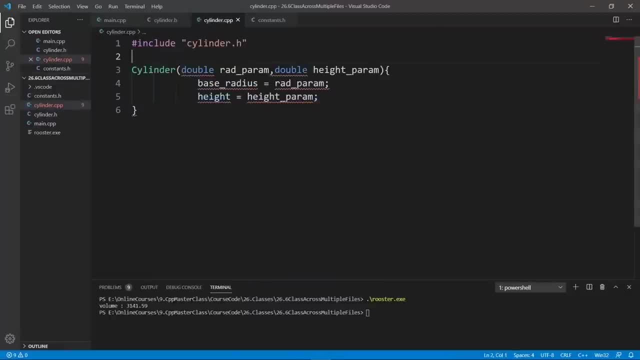 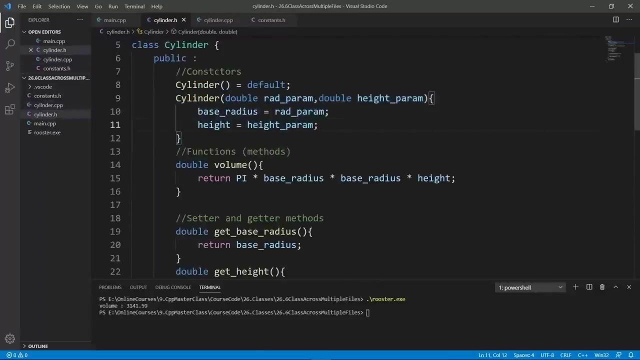 implementation of a function we have in our header here is to put the class name in front. we're going to put two columns. the moment we do that, the compiler is going to know that this is an implementation of a function we have in our header file and this is the function. here and now we can. 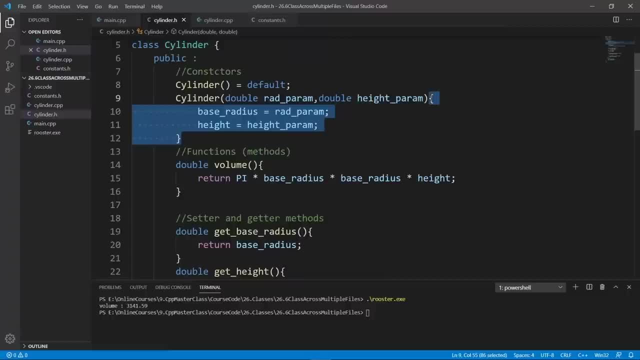 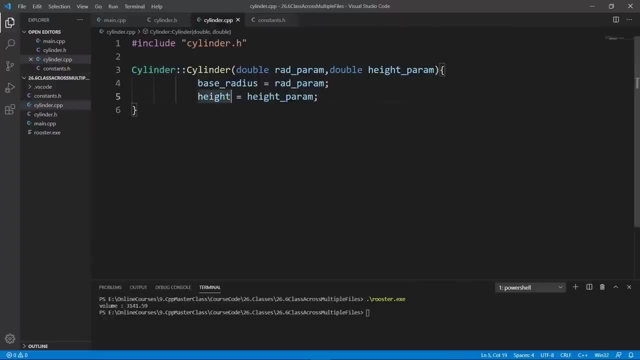 take out the body here and live this as a prototype for the function which is our constructor here. we can do this. okay, if we do this in world, the code is going to build, it's going to construct our objects. let's go back in main cpp and make sure that that's the constructor we are using. it is. 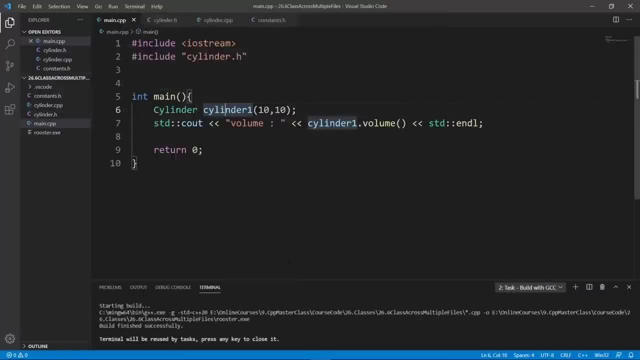 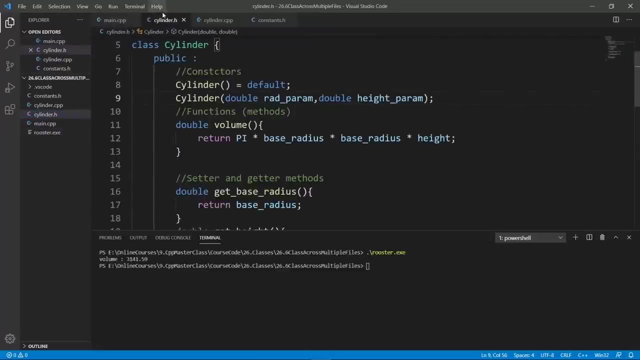 we can bolt and make sure that what we just did didn't break anything. we are building and we can clear things up a little bit and run rooster. this is going to give us our volume and we have started to split things up in our class here. some things are going to leave in the header file, some other 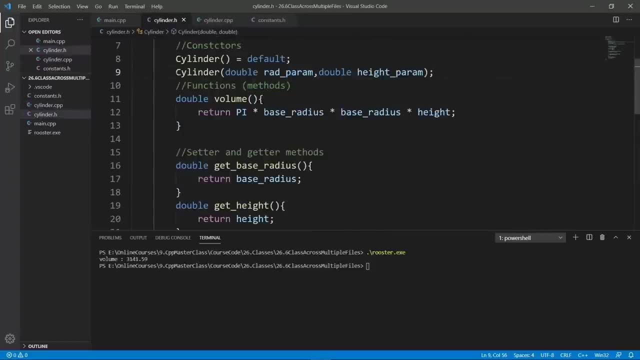 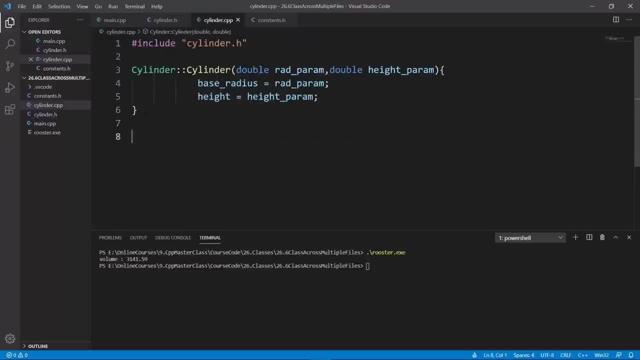 things are going to leave in the implementation file. so we have moved our constructor here. let's move the volume function. we can grab it and move things line by line. i think this is the best way to learn and i think we can move this fence a little bit to the left. let's do that and we're going to. 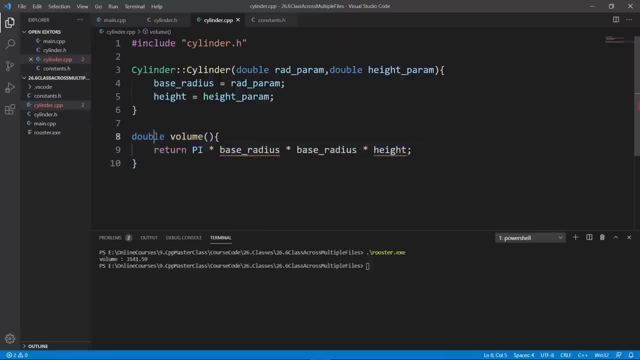 say that this is a function implementation for some function that is declared in the class here. so we're going to say cylinder and we're going to put two columns. this is going to tell the compiler this is an implementation of the function we have in our class and the return type has to. 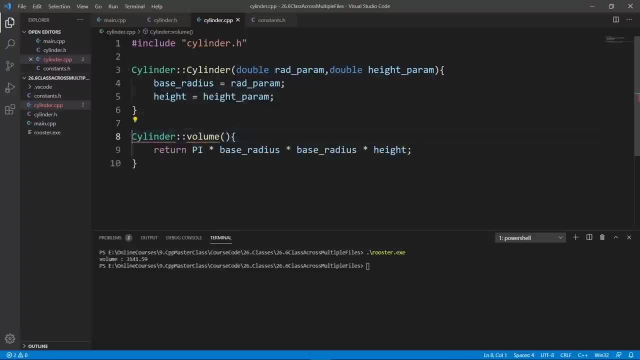 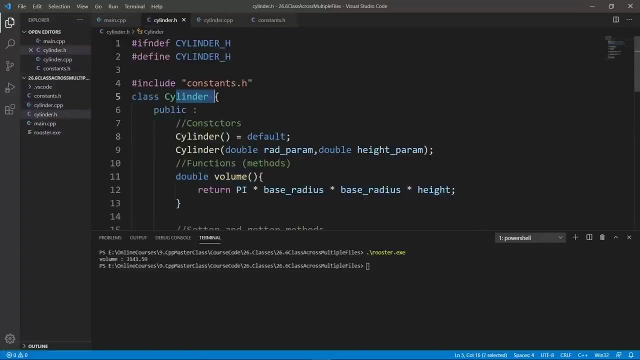 leave in front of this scope resolution operator. okay, what we have here- cylinder colon. colon- is called the scope resolution operator and is basically telling the compiler that our function called volume leaves in the scope of the cylinder class. this is what the syntax here is saying, and this little thing here is called a scope resolution operator. 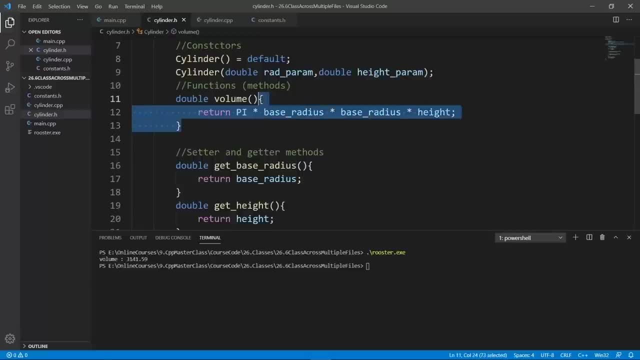 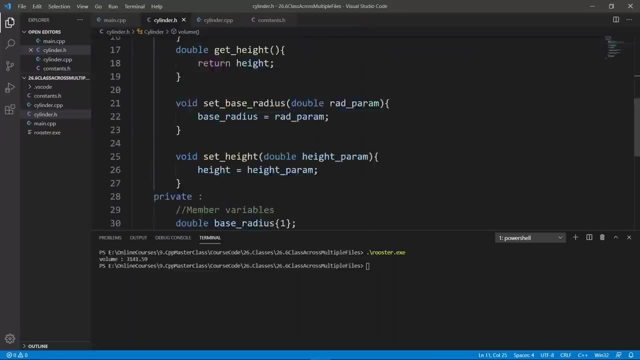 okay, so we have moved our volume function. we can now take the body out from the class and keep the prototype here. we can go down and really practice on the setters and getters. let's do that. so we're going to grab them all together, because now you. 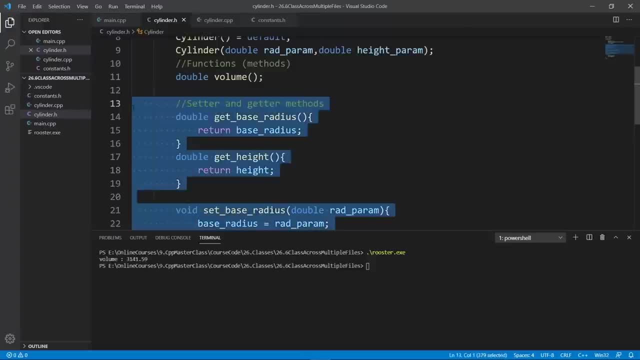 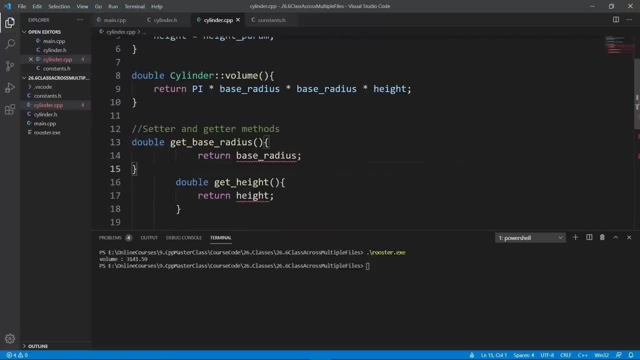 have the gist about how this works. we can copy them and move them into the cpp file, and we're going to fix the code line by line here. so let's make sure they are aligned properly. we have two left to do. let's do that, and i really have to show you this life, because some people are going to have. 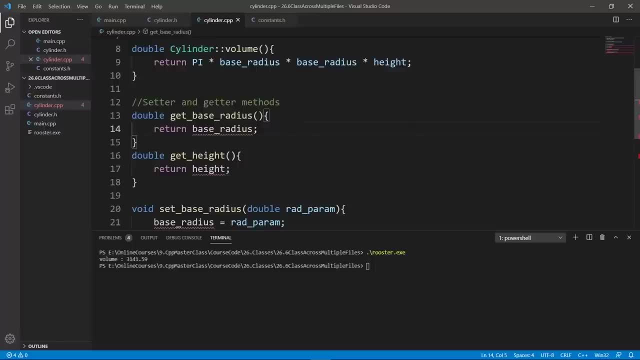 problems regarding how i did this, so i want you to see this live. as i do this, i'm not going to edit this out. so we're going to put our scope resolution operator after our return type here. we're going to say cylinder, cylinder can't type, can i? okay, we have. 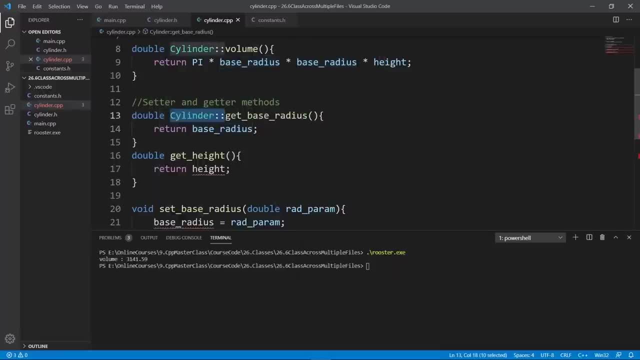 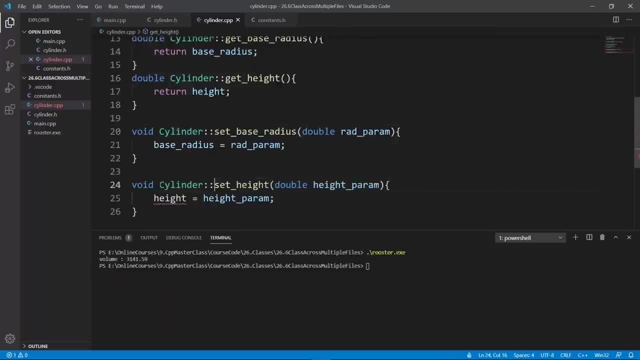 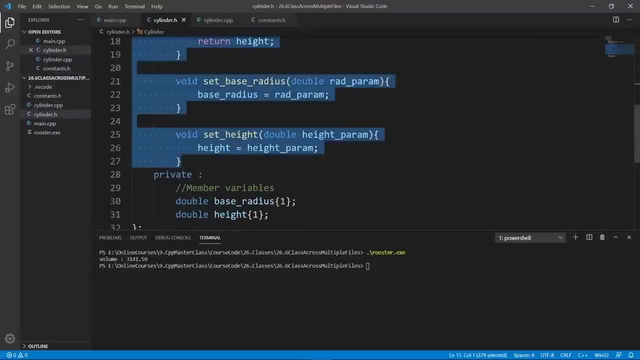 this in and we can really copy this and paste this into place wherever it is needed. so i'm going to paste that here, i am going to paste that here and i am going to paste that here. now we have successfully moved all the functions in the implementation file cylindercpu. 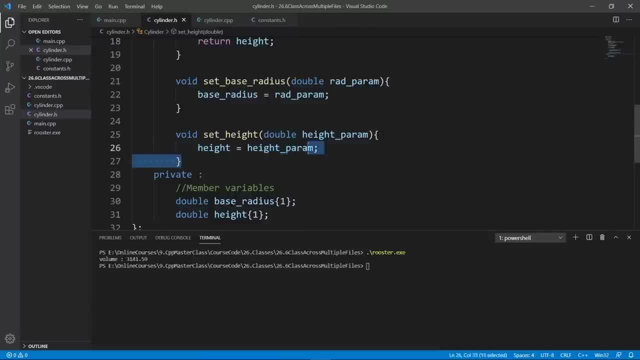 p and we can go back in our header and remove the bodies because we don't need them here. if we keep them here, we're going to have two definitions for this functions and we're going to have compiler errors. let's check this out. we're going to take the body out. 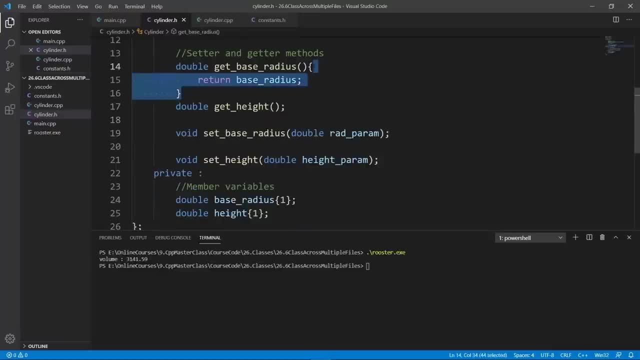 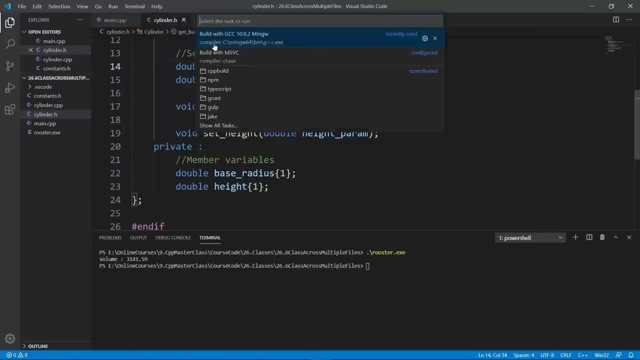 we're going to take the body out and we're going to take the body out. let's do that for a gate base radius, here and now. if we build our program, it should world. we're going to world with gcc. see, the world is good. and if we try to run the program, it should. 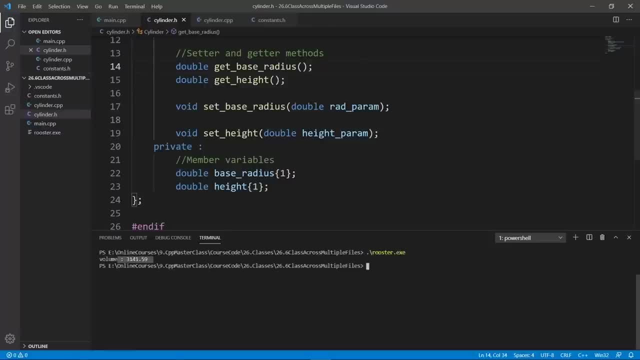 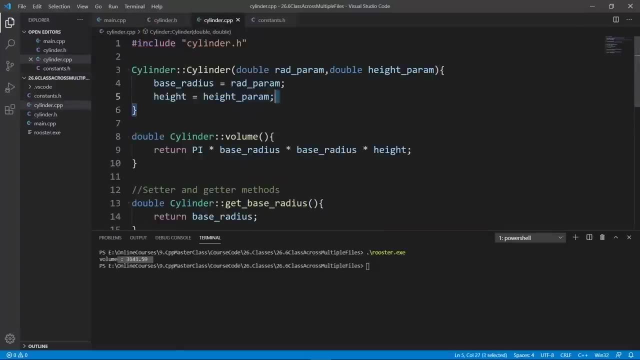 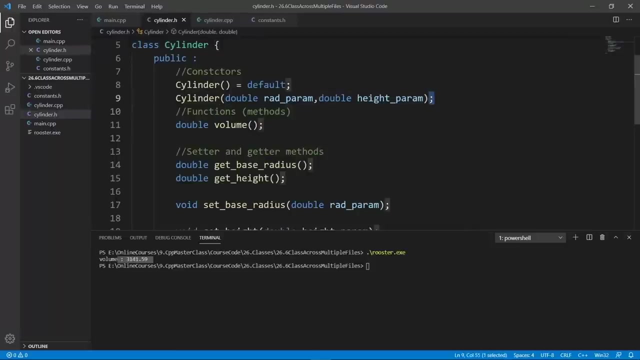 give us what it was given before. this is the volume here. one thing i want you to see is that you don't want to keep two definitions for your functions so, for example, we can grab the body here and bring this back in the header file. i want you to see what's going to happen if you do that. i am 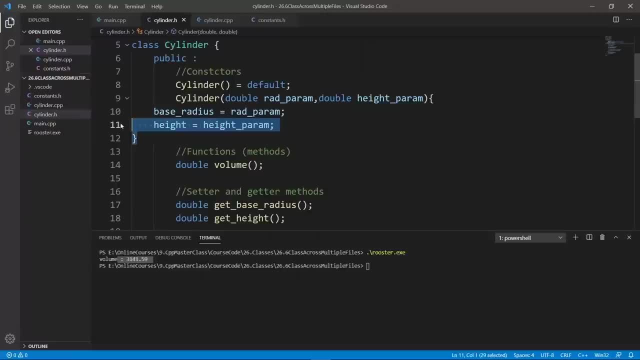 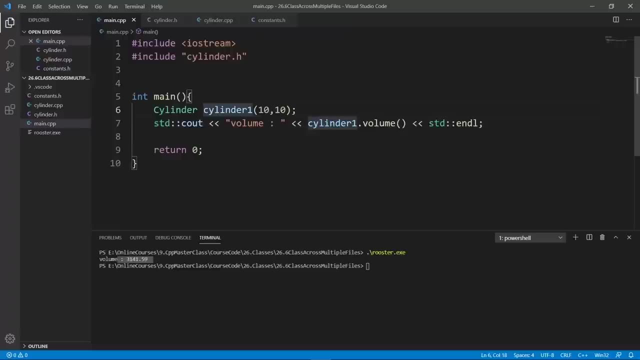 going to paste that in here and i am going to move things a little bit to the right to align things properly here. so if we do this, the compiler is going to see that we are calling that constructor and the compiler is going to have no problem with us. but once we hit the linker stage, the 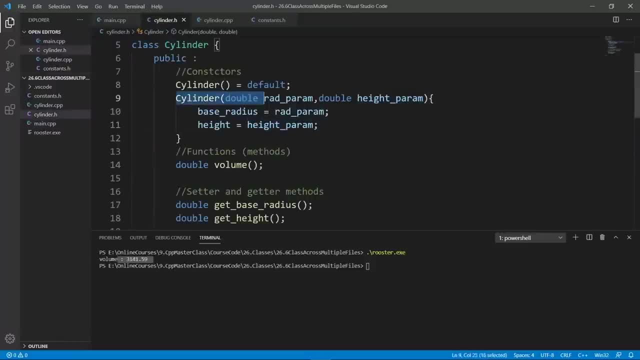 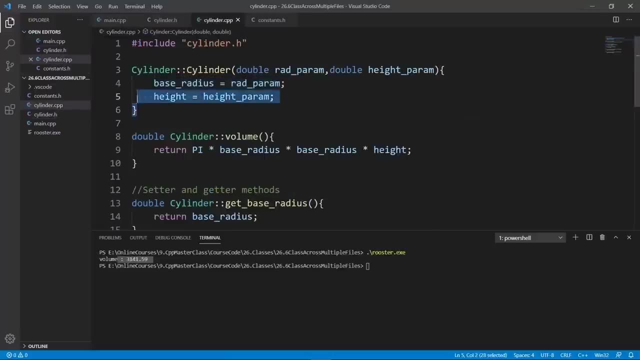 linker is going to find that we have two definitions for the constructor here. we have one in the header and we have one in the implementation file and this is going to raise a compiler error saying we have two definitions for the constructor here and the linker want to. 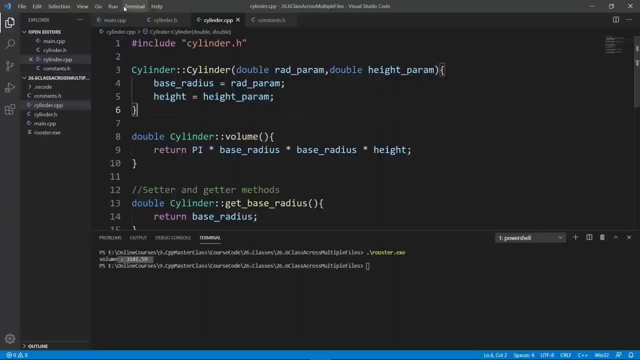 know which one is destroy, because the construction of this constructor is actually annoying. so let's drag out this one into our each instance here and let's take a look at this one and we will see one to use. so it's going to give you an error. let's build and really show you this, because 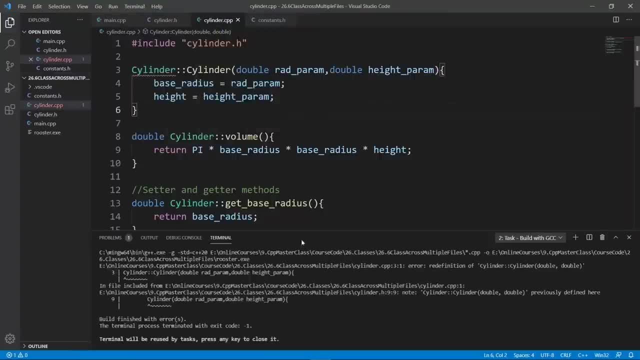 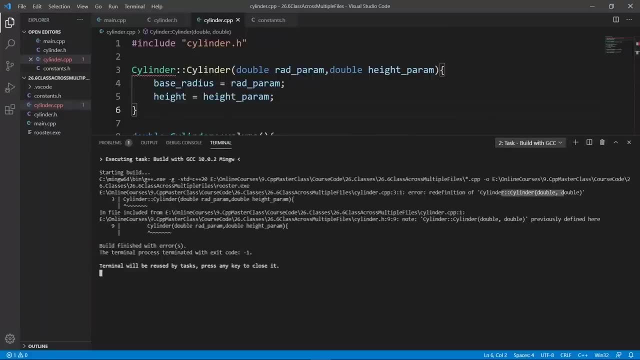 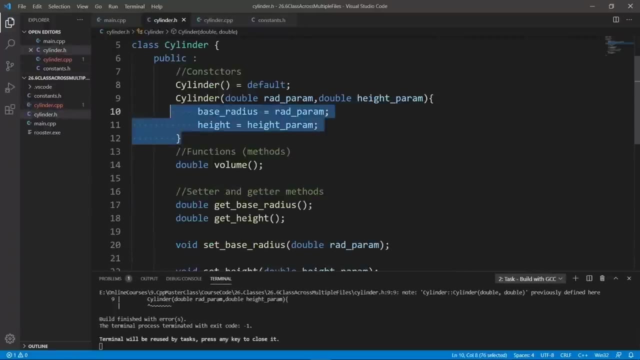 this can be hard to debug if you don't know what is happening. okay, you see, we have world finished with errors and the problem is cylinder. cylinder, double, double is redefined. we don't want to have two definitions for the same function. so once you move things from header to implementation file. 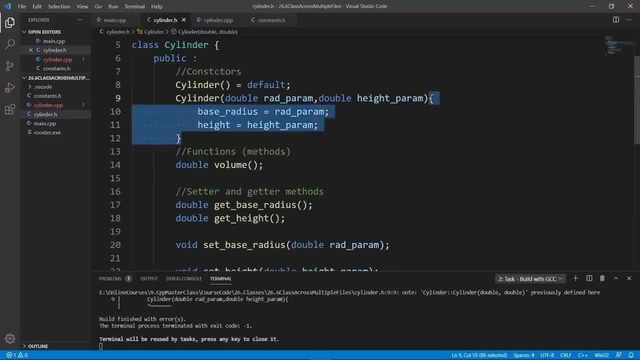 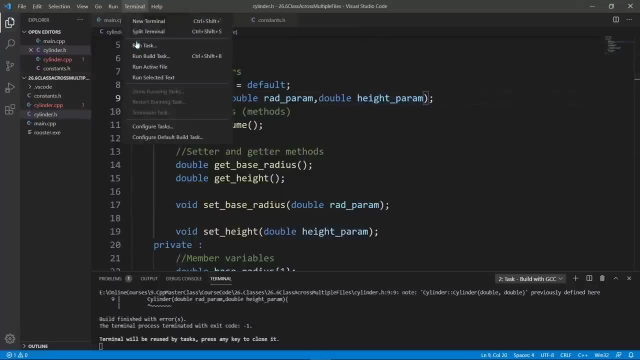 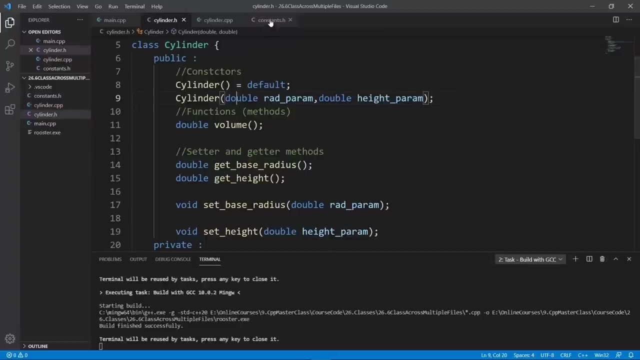 be sure you don't have any more definitions left in the header or you're going to have really hard to debug problems. and now i think we have our program organized fairly well for what we know so far about c plus plus. we have our constants living in another header file and we have learned. 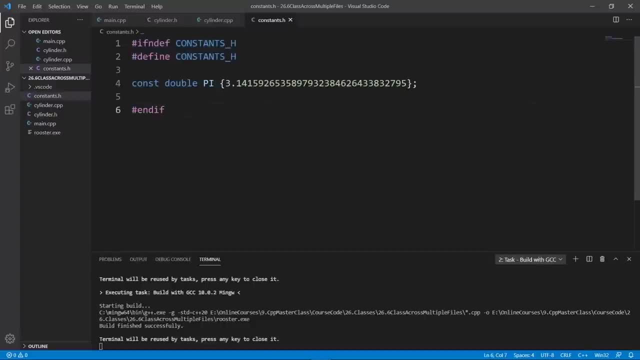 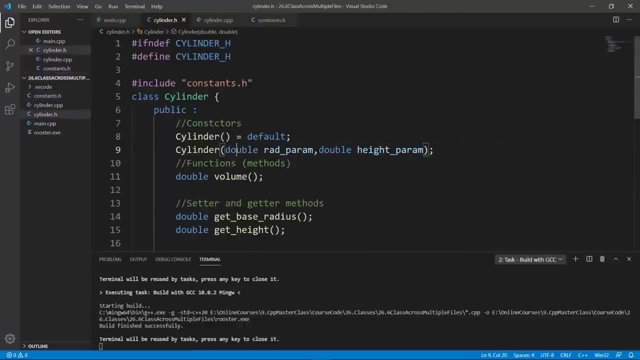 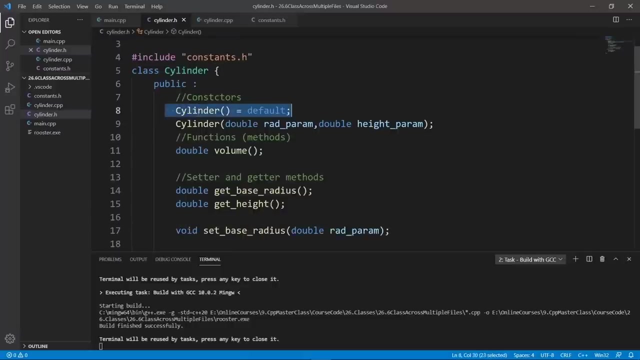 about include guards, what we can use to guard against our stuff being included more than once by the preprocessor. we have our cylinder class living in its own file and again we have an include guard here and you can see that this class now is really easy to look at. we can look at the information about the member functions. we 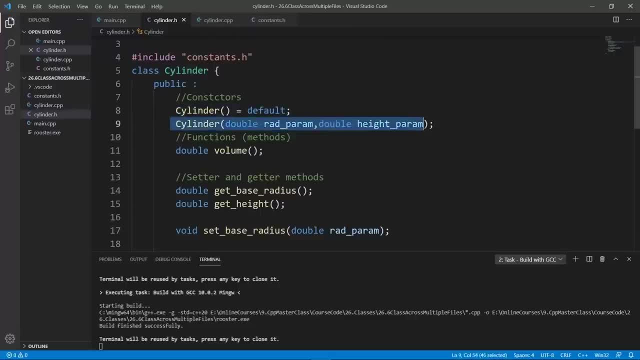 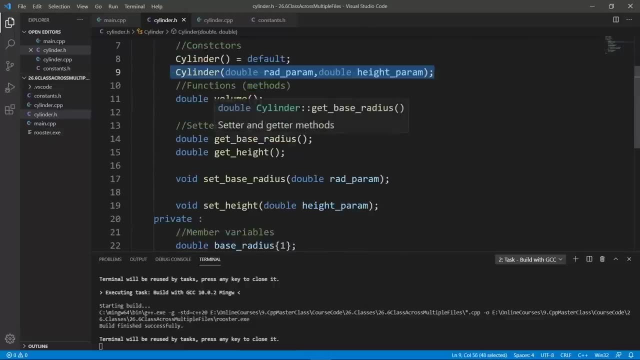 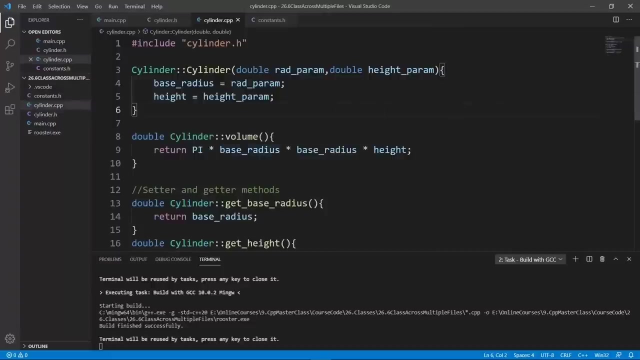 have. for example, we have a default constructor, we have a constructor that takes two parameters, but we don't see the details about how these things do their jobs. for example, we don't see the details about how the volume is computed. those details are hidden in the cpp file and, if you want, 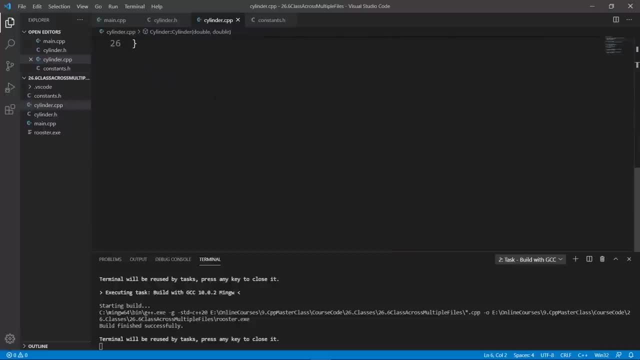 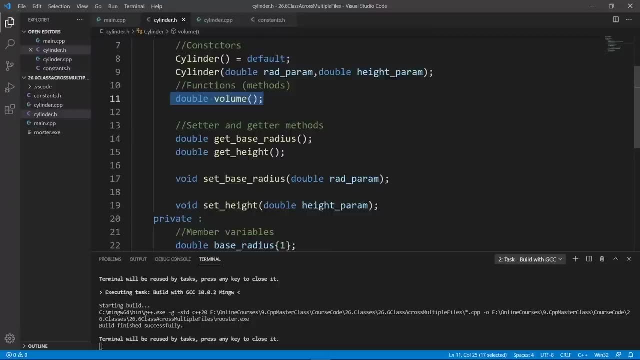 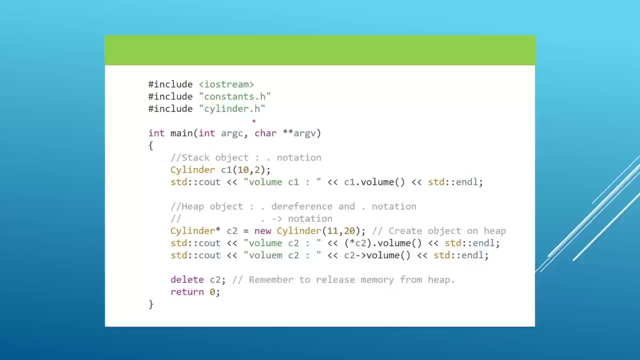 to see them. you need to go to this implementation file here. this is a good design and i encourage to split your c plus plus programs in multiple files like this. this is going to make your life easier. in this lecture, we're going to see how we can manage our class objects through pointers and 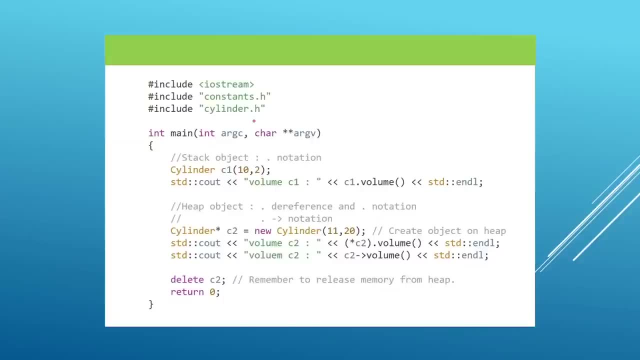 in most cases we need to manage our class object through pointers if we are using some form of dynamic memory allocation. here is a simple example. we have our cylinder class included and down here you see that we can create cylinder objects on the stack if we use the syntax like we. 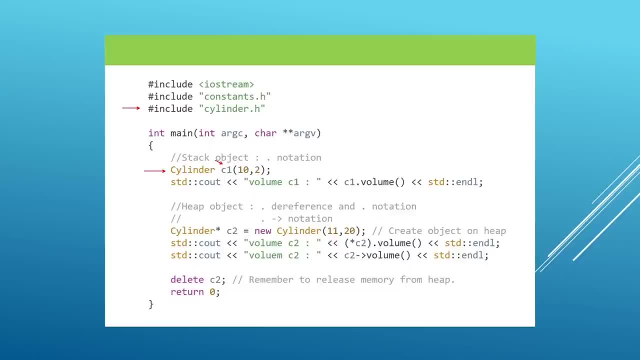 do here. the objects are going to be created on the stack and we have seen that we can access the behaviors or data inside our class object using the data notation, like we do here. for example, here we are calling our volume function, but sometimes we want to manage our objects. 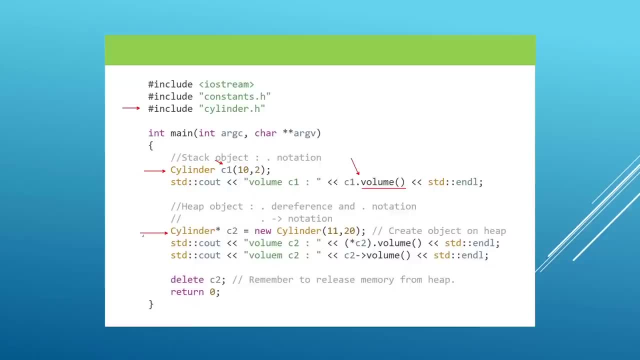 through pointers. for example, if you look at the syntax we have here, we are saying cylinder and using the asterisk here. this is going to say that this is going to be a pointer to a cylinder type and i'm going to give it a name, c2, and we can allocate our object on the heap using the new. 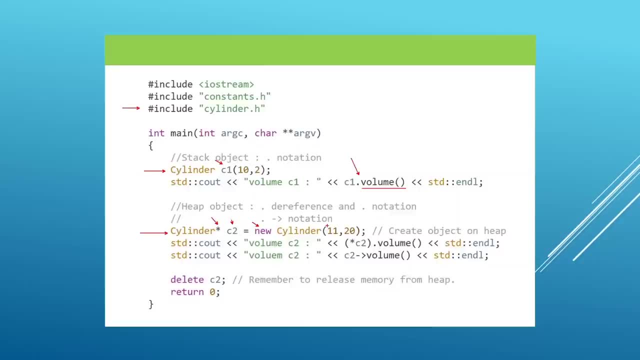 operator. this is going to dynamically allocate space from the heap and that memory space is going to be used to store our cylinder object. now the interesting thing is going to happen. when you try to access behaviors from the c, c plus folder, you can see that when you access behaviors from the 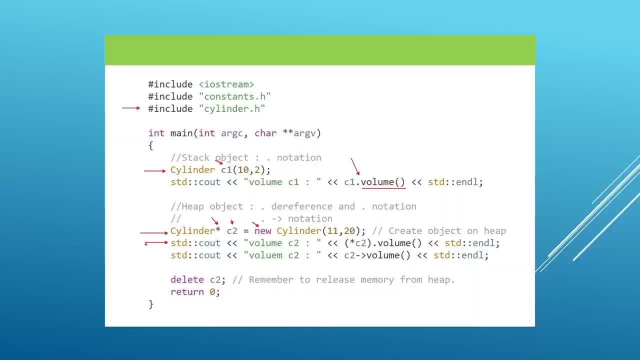 your cylinder object. here, for example, if we look at this line here we are trying to print the volume of this cylinder and you notice that we have to go through ugly, the referencing. here we have to the reference, the object, and then call our method through the dot operator here. but what i want you 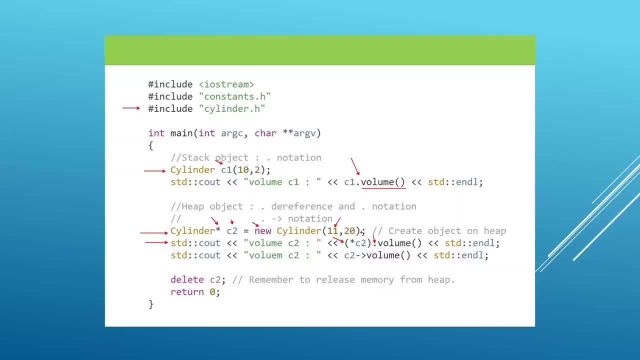 to see is that we can avoid this ugly, the reference that we are doing here, and use the pointer access notation. this dash, greater than symbol you see here is going to allow us to access stuff directly using the pointer to an object that is dynamically allocated on the heap. 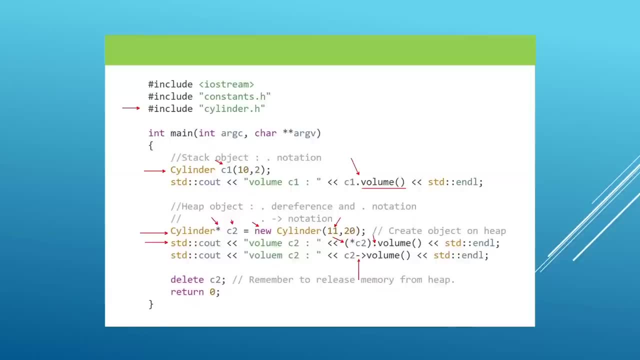 okay, after we are done using our cylinder object- remember it is memory that was dynamically allocated from the heap- we have to release the memory so that it can be used by the operating system, and we release the memory using the delete operator, as we do here. okay, the idea i wanted to introduce here is that we can use pointers to manage our cylinder objects. 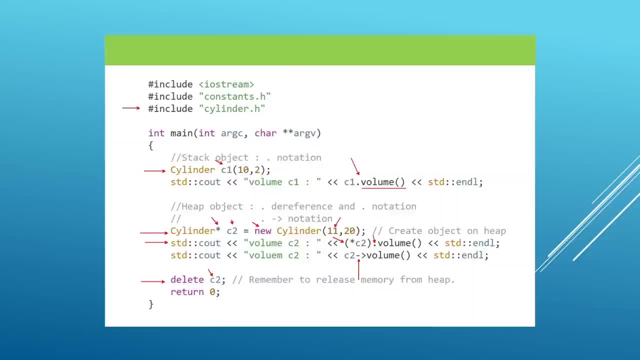 and this is one way we can do this. and once we are using a pointer as a handle to our cylinder object, we can use the pointer access operator here to access stuff from our class objects easily. and another thing you should know is that we can actually create a cylinder object. 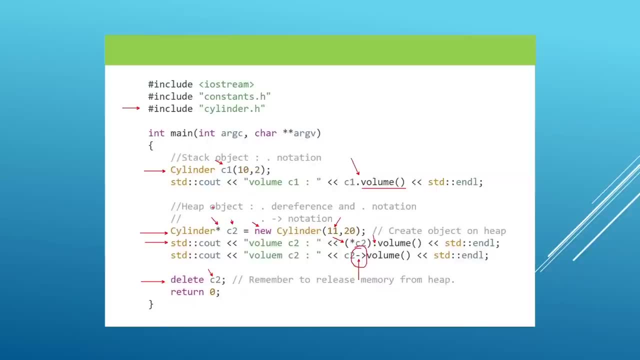 and store in the address of objects that we have on the stack, and we're going to see this in a minute when we hit visual studio code. now that you have an idea about this, let's head over to visual studio code and play with this a little more. okay, here we are. 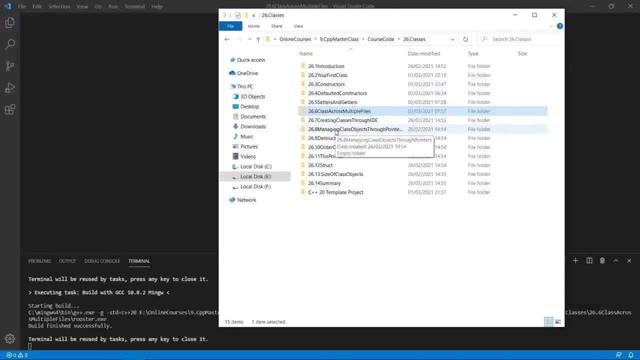 in our working folder. the current project is managing class objects through pointers. we can see the entire name here and now. we're not going to grab our template project because we want to start from the project we had in this lecture on class across multiple files. so we're going to go. 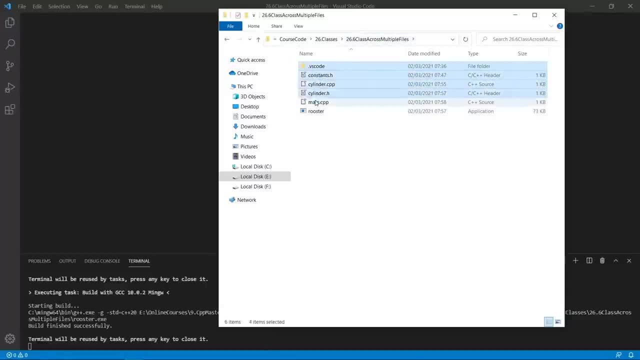 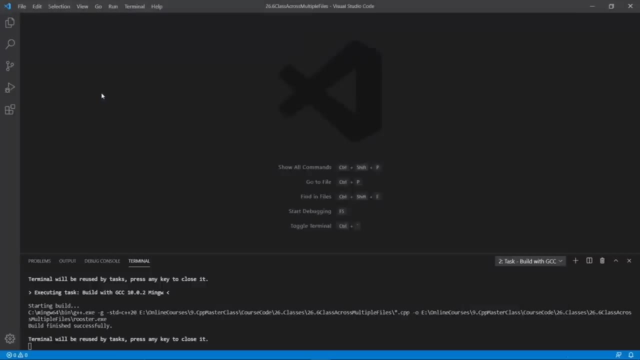 in that project and grab everything from there except for the executable, because we obviously don't want this and we're going to go in our current project and paste in the code and this is going to give us a good starting point so we can grab this and open this project in visual. 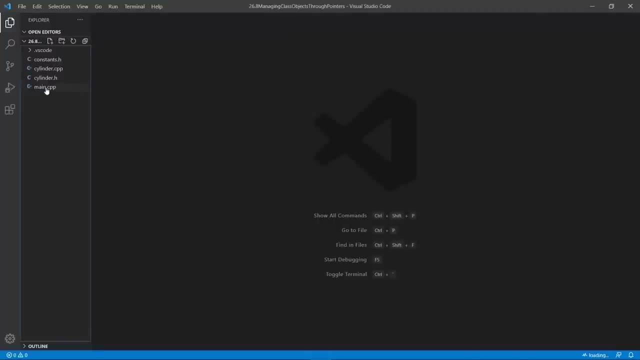 studio code. it's going to open the folder and we're going to have everything we want to start doing what we want to do in this lecture here. so now we should have access to our cylinder class and if you look here we have an object of cylinder type already created by this line, on line number. 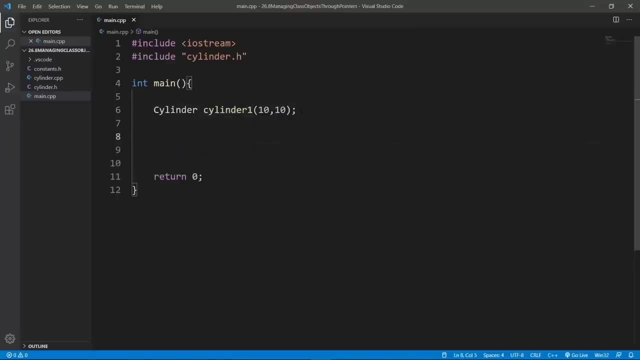 six here and we have seen that we can use the syntax like cylinder volume here, using the dot call operator to access stuff from our class object and this is going to work. but we want to see that we can use pointers to manage our object here and the first thing i want you to see is that 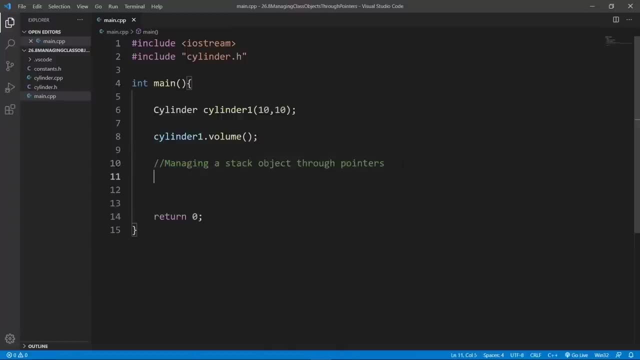 we can manage a stack object through pointers, and that's what we're going to do in this lecture. to really show this off, let's set up a another variable. it's going to be a cylinder pointer and it's going to be p cylinder one. it's going to be a pointer to cylinder one here. that's what. 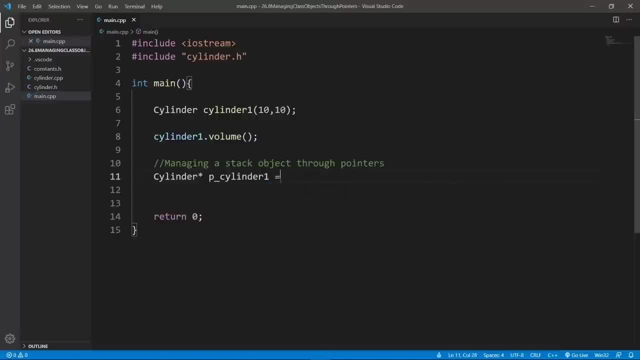 i mean, and we can give it an address of cylinder one as a value, so we can do that, for example, and put in the address of operator, and this is going to work. now we can go through our pointer here and do stuff with this cylinder object, but the syntax is going to be pretty ugly. so for 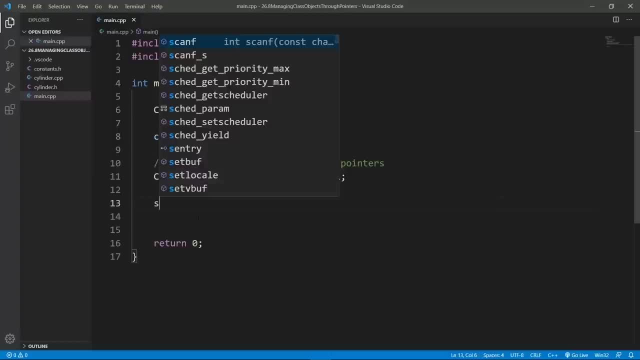 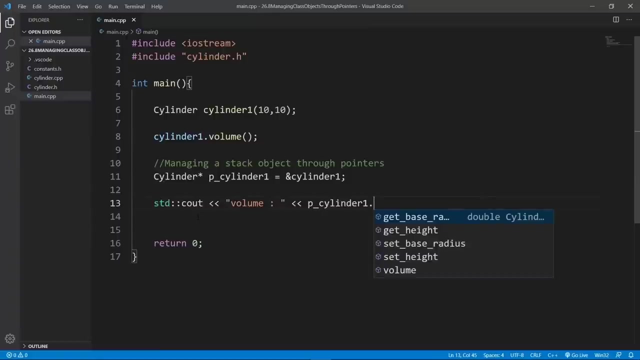 example, let's try and print the volume of our cylinder. we're going to say sdc out and say volume can say that and we're going to have to go through the reference operator. so if we do something like p cylinder one and try to use the dot operator, you're going to see that we have the volume. 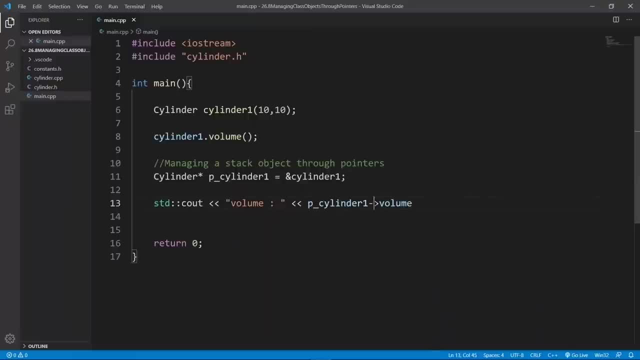 function. but if we try to call it, let's do that, let's make sure we are using the dot operator here. if we try to compile this program, it's not going to be the dot operator, but it's going to be the dot operator because we are trying to call stuff from a pointer and remember: a pointer is just. 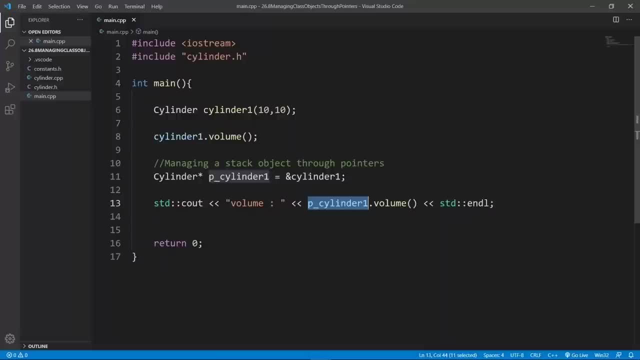 going to store an address, it doesn't really have information about the type that it is pointing to. if we try to compile this program, we're going to get a compiler error, so let's use jcc to do that- and we're going to get request for member volume in p cylinder 1.. remember, p cylinder 1 is just a. 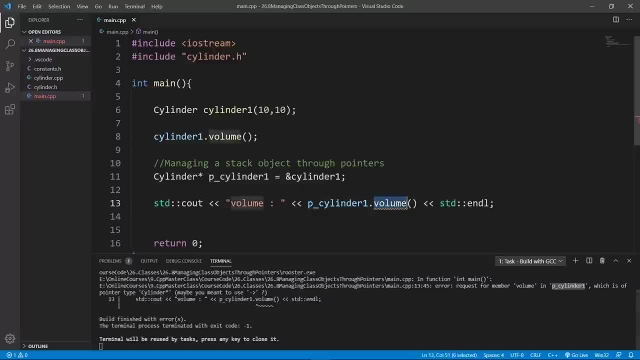 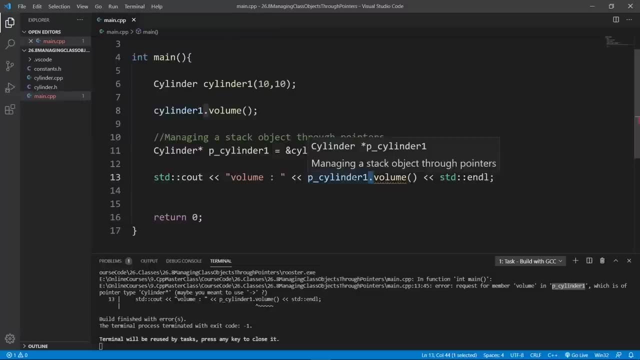 pointer. it's not an object, so we can't really call the value of p cylinder one, so we can't really call the volume function to it. if we want to use the dot call operator here we have to dereference and actually get to the actual object that the pointer is pointing to, and we do that using the star. 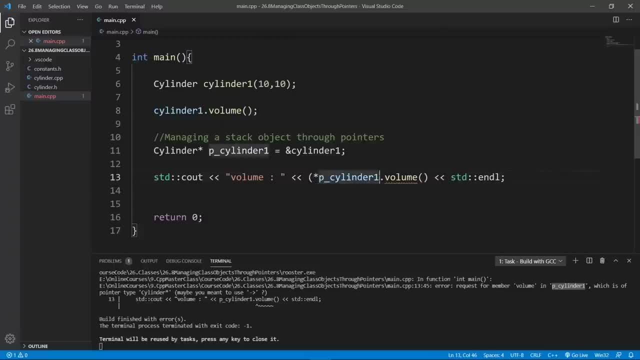 operator. you already know how to dereference a pointer, so we can dereference our pointer and then call the volume function on what the pointer is pointing to, and this is going to work. it's going to print our volume. let's build now, now that we are dereferencing correctly, and you see that this is. 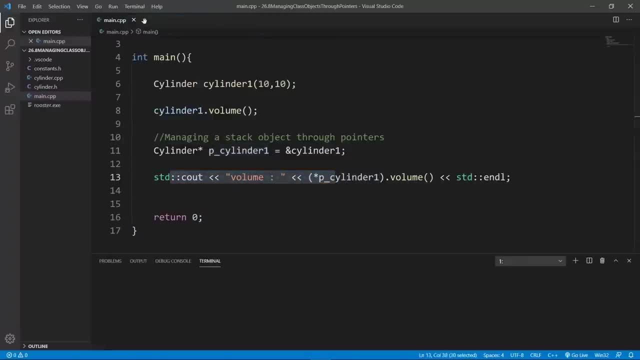 going to work. and if we try to print this, let's bring up a terminal so that we can run this program. let's run roaster. you're going to see that we have our volume here. so to really get to what is pointed to, you need to use the reference operator and then call whatever method you. 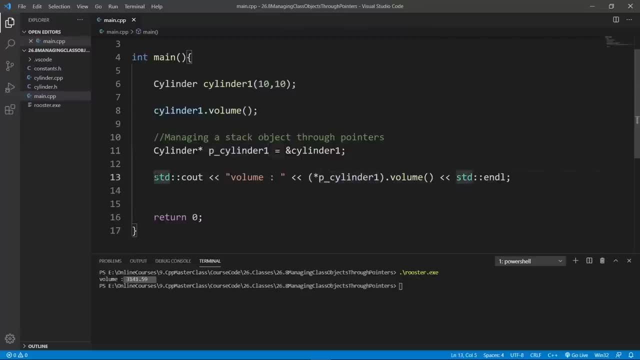 want to call on your object. but we can do things even easier. there is a syntax we can use to use the pointer directly here, because going through all this, the referencing ugliness, is really not cool. so we're going to grab this and show you that we can use the dash greater than operator. 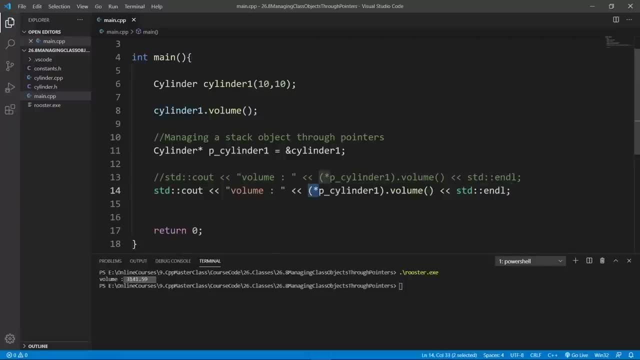 that's how i call it and if we use that, we don't need to the reference. all we need to do is use the dash greater than symbol here and it's going to directly tell the compiler: don't call stuff on the pointer directly. do the reference the pointer internally and then call the volume function. 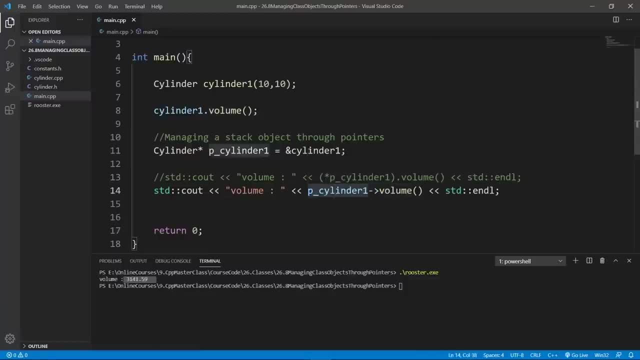 on whatever you get after the reference then. so this is basically going to push the referencing ugliness here behind the curtains of the compiler and we can use a nice syntax like this, and i think this is much better than what we were doing here. so if we try to bolt now, we're going to bolt and print our volume, you're going. 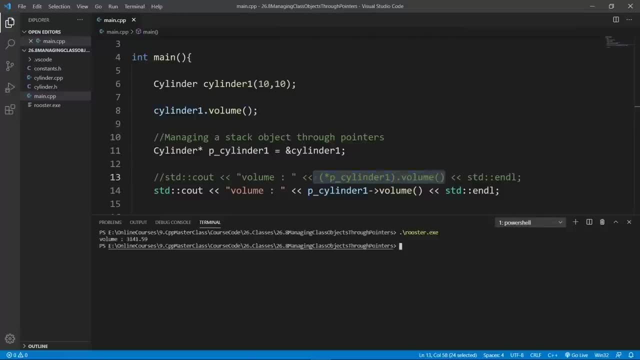 to see. the world is good. you can clear and run rooster. you see, we see our volume here. so this is what i want you to see. it is possible to manage your cylinder up objects through pointers, and this is one way we can do this: by managing a stack object through. 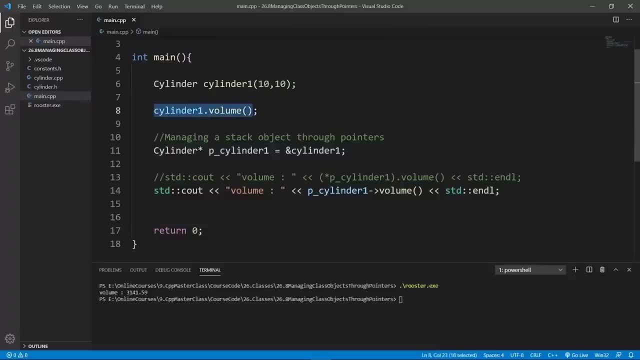 pointers, and this is what we are doing here. if you want to call stuff on your class object, you can either do the ugly stuff we do here or you can use the nice pointer access operator and it is going to be cool. okay, now that we have seen this, let's see another use case in which we're 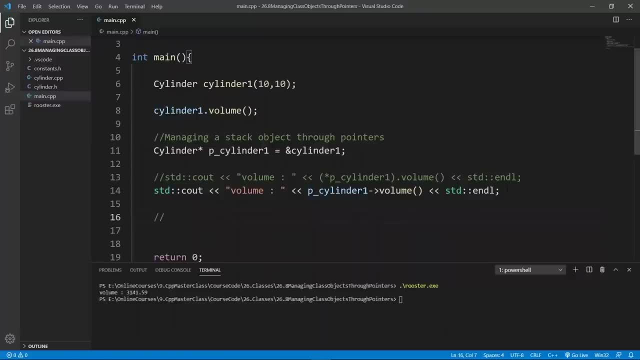 going to be creating a cylinder object on the heap through the new operator. okay, we can go down and save that. we're going to say cylinder pointer. it's going to be p c, lender 2.. we can call it like this. and then we're going to say new cylinder and you're going to see that we can call. 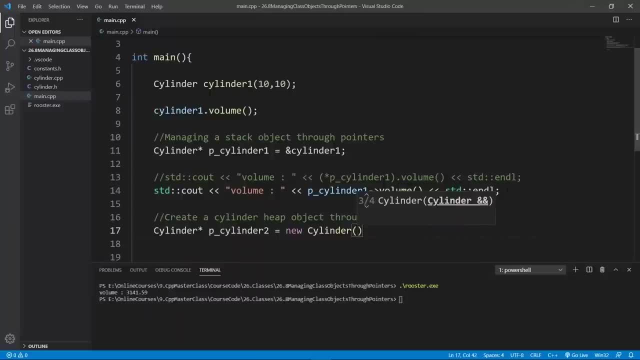 a constructor. we have two types of constructors. we can call we're going to call our constructor. that takes two parameters, and we can pass in 100 and 100- why not? oh, let's put a 2 after here. we can put in whatever we want. this is going to create a new. 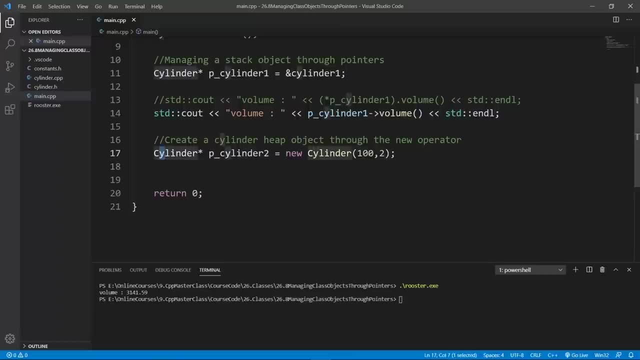 cylinder object. the space for the cylinder object is going to be allocated on the heap, so this is a heap object and because we are using the new operator here, the other thing you should have in mind is that you will need to release this memory, and let's go and do that directly. this. 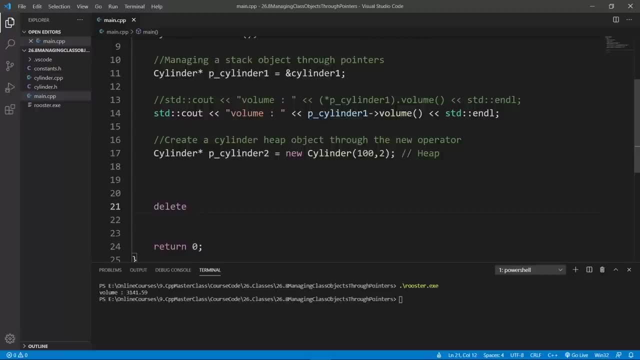 is a good practice, because you will forget to release your memory if you don't really keep this in mind. so we are going to delete p cylinder 2, because that's what we used to allocate our heap memory here. okay, now that we have taken care of memory management, we can go in and use our p cylinder. 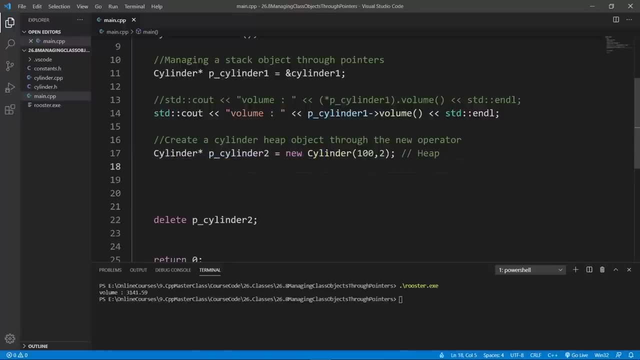 2 object and, for example, we can print its volume by using the std c out statement here. so let's go down and save that, let's align this properly, and we're going to say volume, cylinder 2, to really make this super clear. and then we're going to say p, cylinder 2, and call the volume function here. 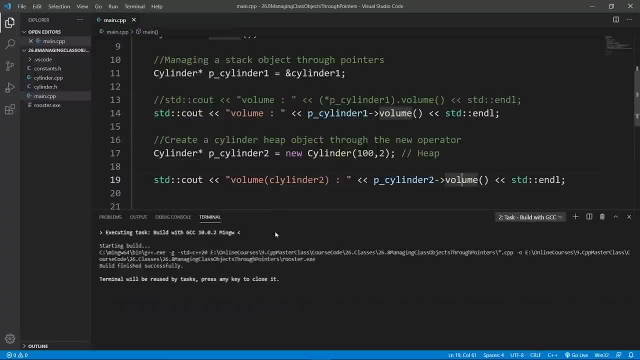 this is going to work. let's draw and the world is good. we can clear and run rooster. this is going to give us our volume and if we try and use this information to create a cylinder, we're going to see that the volume is what we 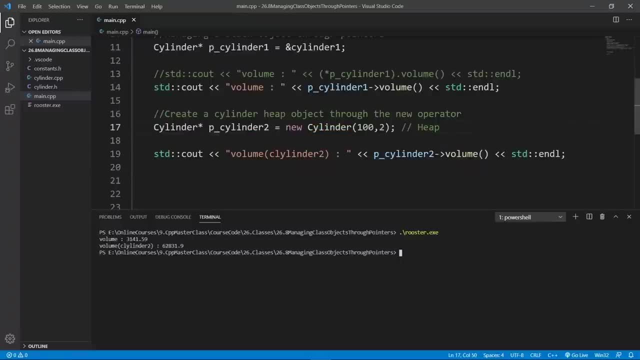 see, here we can even try and print its base radius. let's do that. we're going to say std cl, we're going to say p, cylinder 2, and we're going to say base radius. we can hit the dot operator here. you're going to see, we're going to have a few options in a visual studio code here. 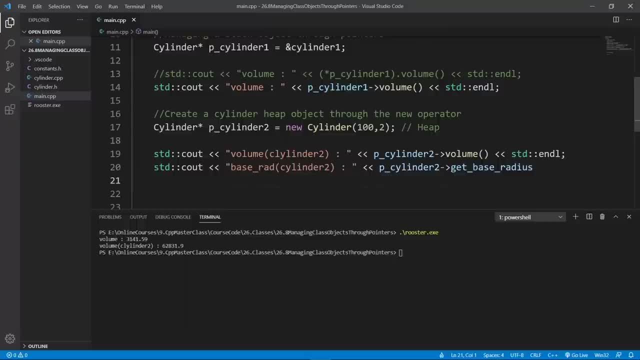 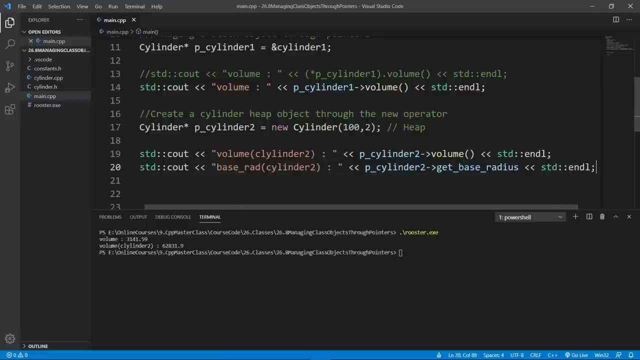 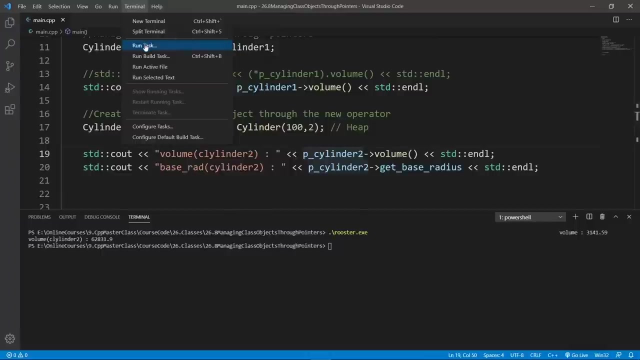 if we double click on get base radius here, you're going to see that visual studio code is going to use the pointer access operator here and this is really cool so we can height std ndl. we can close the left pane here because we need some more breathing space, and if we try to weld and run, 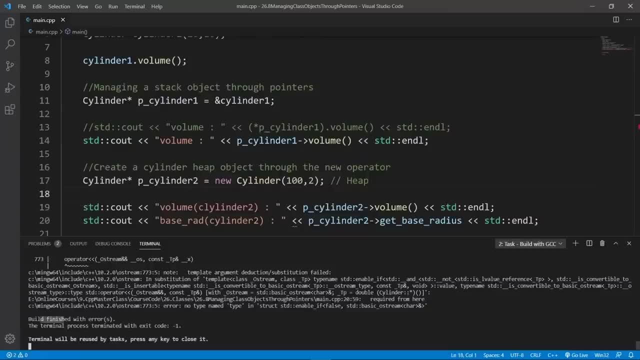 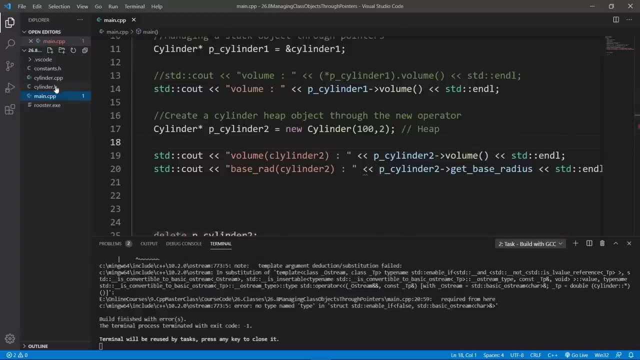 this program and we have a compiler error here and the reason is: get base radius is a function. if we go back in our cylinder class we see that we don't have any dances here. we have nós for the that we have a function called the gate base radius. so if we want to call this in the main, 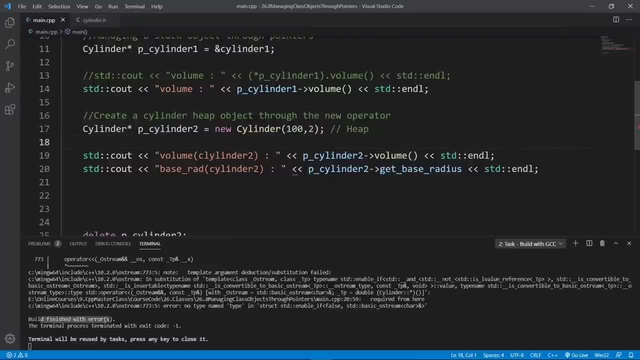 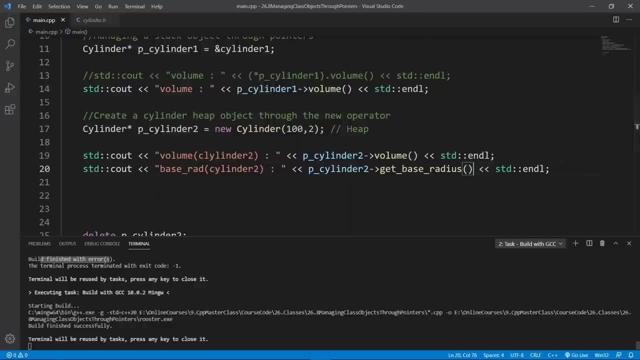 function. we need to call that as a function. so we need to put a pair of parentheses here. and if we build, we should build without a problem. let's do that again. you see, the build is good and if we run the program, we're going to see exactly what we expect. let's run a rooster, we're going to see. 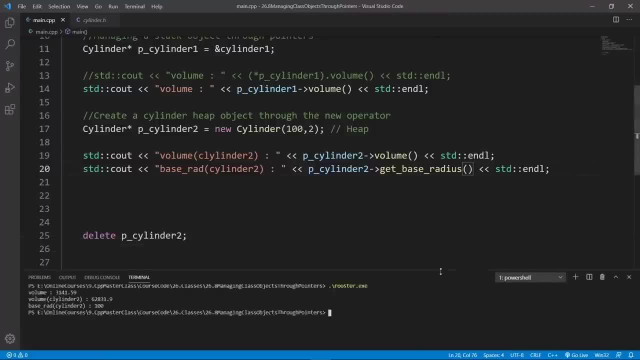 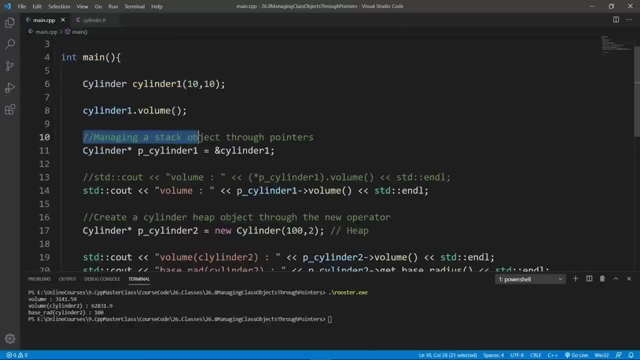 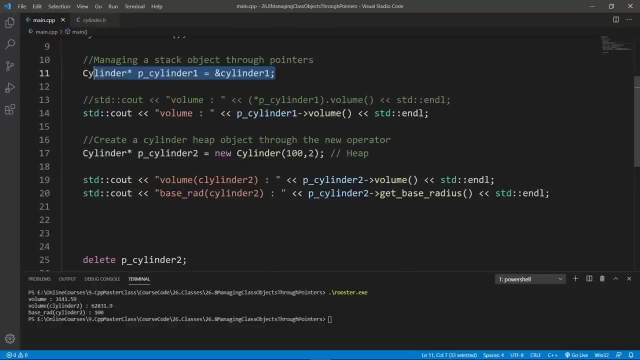 what we expect here and the message here was really that you can manage your class object through pointers. one case is when you have a pointer that is pointing to a stack object, and we saw that we could do that here. we can also use pointer notation to allocate objects on the heap. 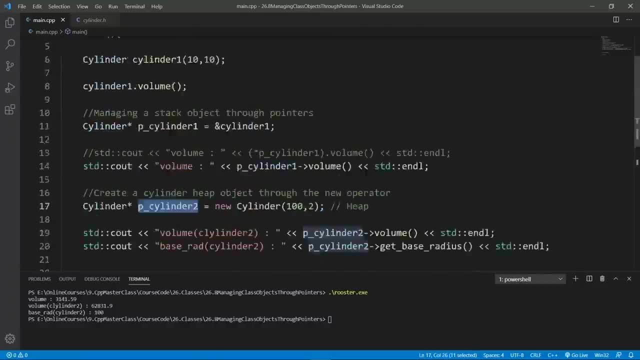 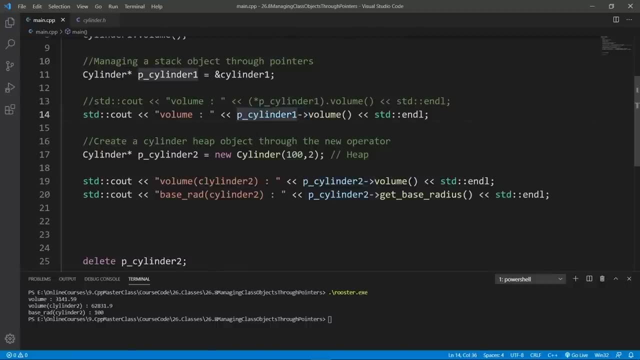 and point to them with our pointer. here, and whenever we are using a pointer, we have the option to use the pointer call operator here to do things easily. i am going to be calling this the pointer call operator to mean this from here on, if we happen to need this, and you should know what i mean by that. this is really all i set out to share in this. 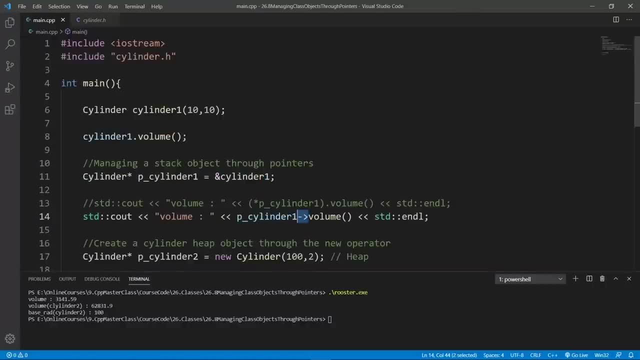 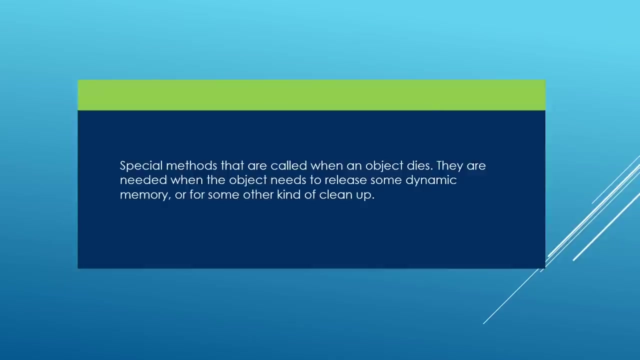 lecture. i hope you found it interesting. we are going to stop here in this lecture. in the next one we're going to learn about destructors. go ahead and finish up here and meet me there. in this lecture we're going to learn about destructors. destructors are spatial functions or methods. in 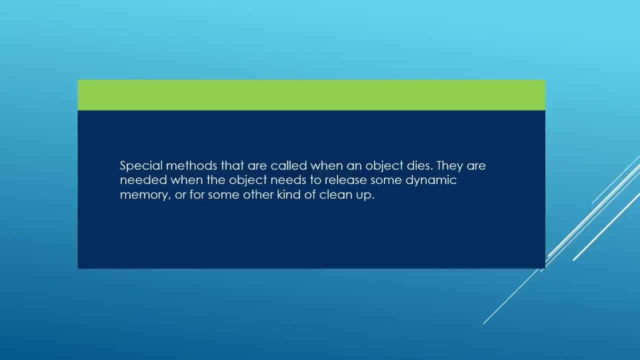 a class and we're going to learn about them in a class, and we're going to learn about them in a class that are called by the compiler to destroy your object, and these are going to be especially useful if you are, for example, allocating memory in your constructors. let's look at a simple example. 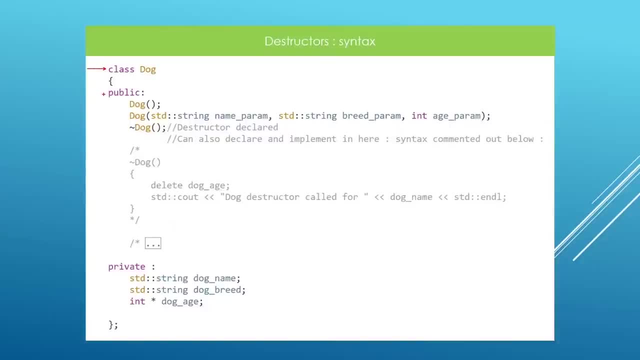 here we have a class called dog. it has two sections: the public section and the private section. in the public section we have two constructors: a default constructor that doesn't take any parameter and a constructor that takes two parameters, and the parameters are going to be used to initialize our member variables, and they are: 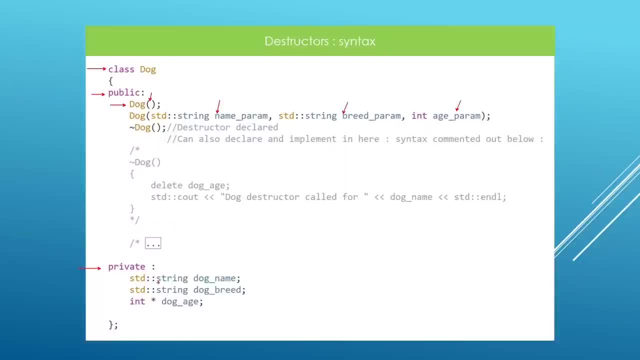 passed by a value here for simplicity, and they are going to be used to initialize these member variables: dog name, dog breed and dog age. the special thing about this class is that it has a destructor and you declare the destructor using this syntax. here it puts a tilde character in. 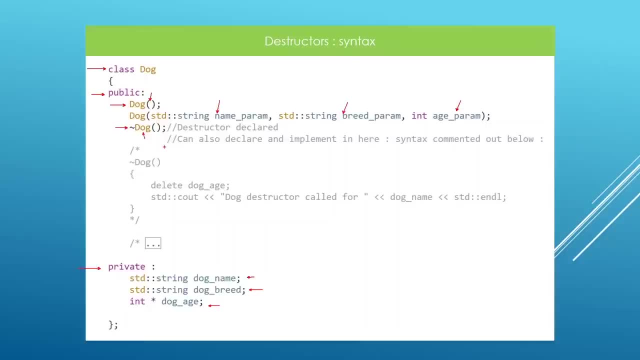 front, you say the name of the class and then you put an empty parameter and then you put an empty parameter last. it is also possible to declare a destructor and put in its entire body in the header, and this is the syntax to do this inside the body you're going to do whatever it is you. 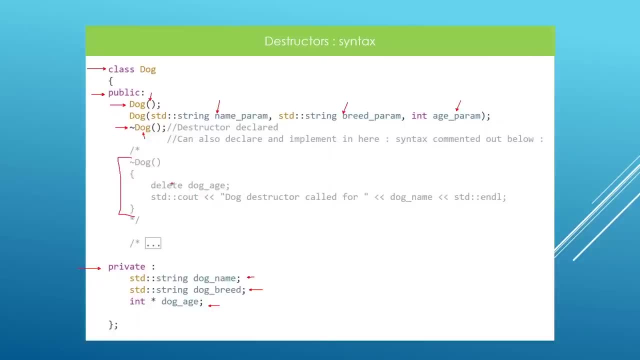 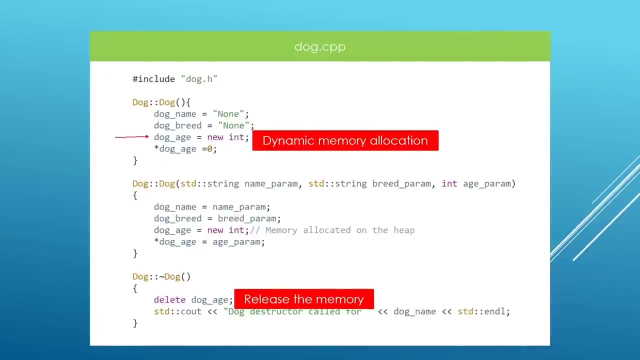 need to destroy your object. for example, if the class here is allocating some memory in the constructor, the destructor is the best place to release that, and this is an example of how you can do that. here is a more direct example of how we allocate for dynamic memory in the. 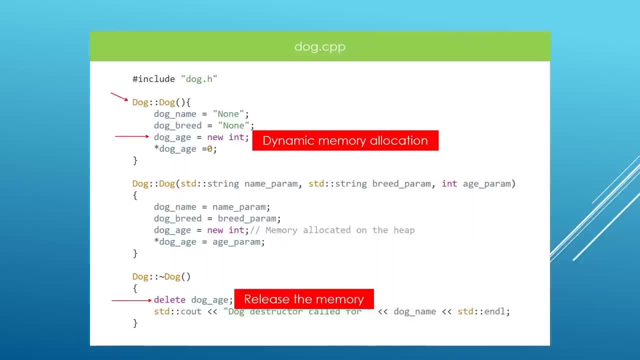 constructor and release that memory in the destructor. we have our three variables but we have chosen to allocate our dog age variable on the heap using dynamic memory allocation and after we dynamically allocate a piece of memory to store our age variable, we're going to set that to zero. 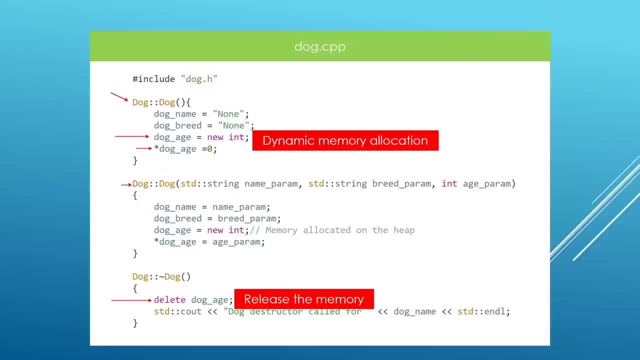 because we are in a constructor. if we are using the three param constructor here, we might use the past parameter to initialize our age variable. but the important thing here is that it is being dynamically allocated memory on the hip here and when our object dies we need to remember to release that memory and the destructor. 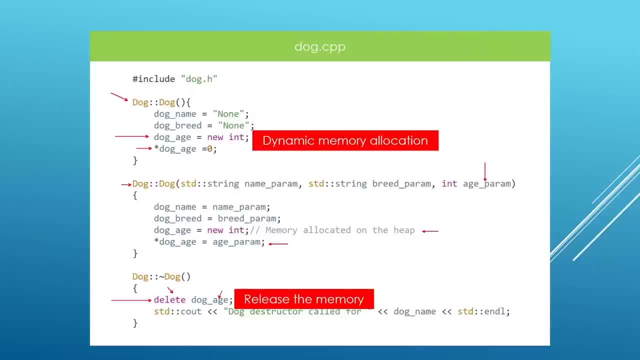 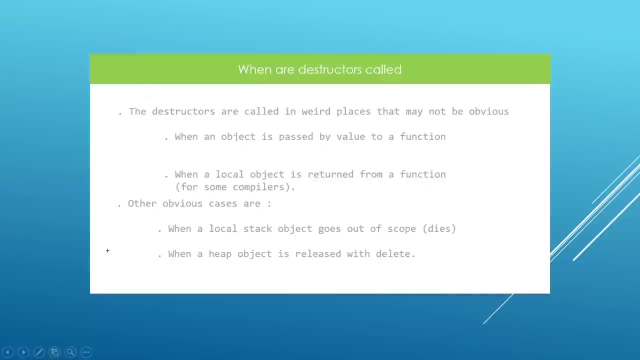 is the best place to release that memory. as you see, here we say delete dog age when our object dies, and the compiler is going to call this function when it's about to kill the object. so you might ask: when are destructors really called? we are going to start by looking at obvious cases here, for 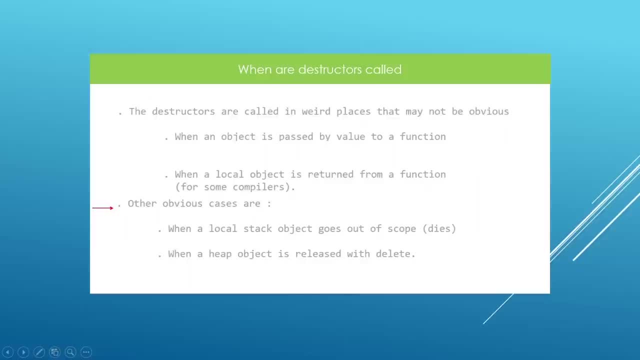 example, when a local stack object goes out of scope, the destructor is going to be called because that object is going to be wiped out from memory. so this is an obvious case in which the compiler will need to call a destructor. also, when a heap object is released from memory using delete the 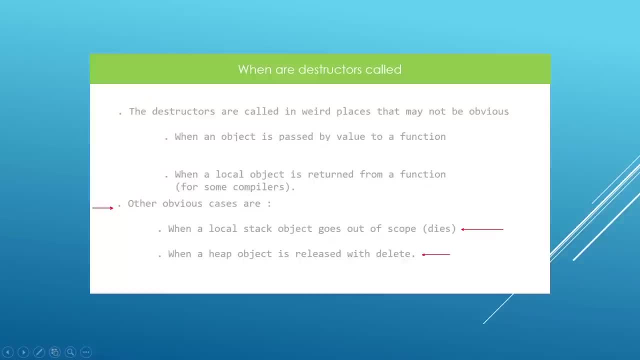 destructor is also going to be called. but there are some indirect ways in which destructors are also called. for example, when an object is passed by value to a function, this is going to call the destructor to kill the object. when the object goes out of scope in the 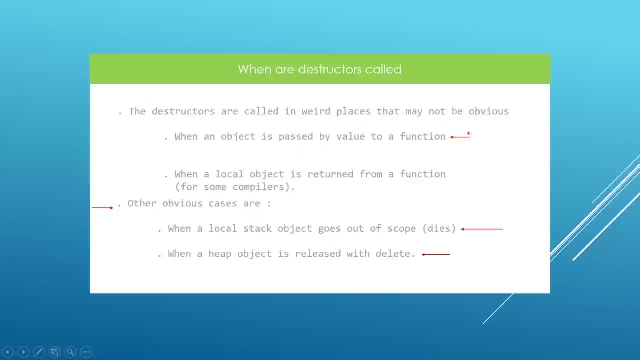 function, because when an object is passed by value, we're going to have a copy in the local scope of the function and when the function exits, that local copy is going to be killed and we're going to see an example of that. another case where you might have the destructor called is when a local 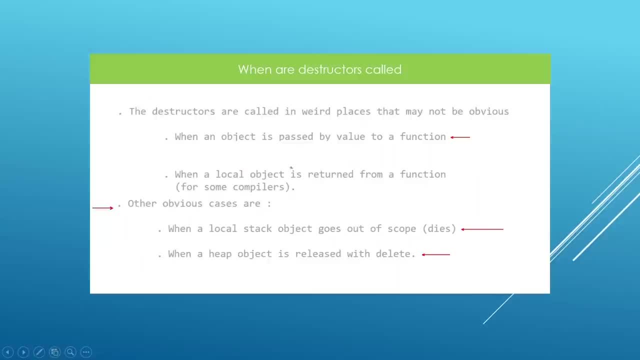 object is returned from a function, another copy is going to be created to be used outside the function and the copy inside the function is going to be killed. but this is not guaranteed, as some compiler may optimize your return value and use some kind of reference. so you're not guaranteed. 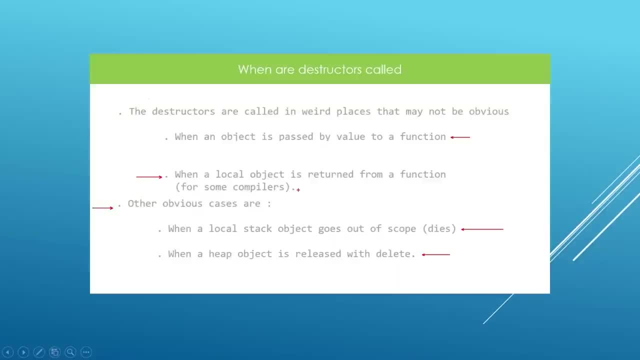 to see this behavior, but it is possible to see it. now that you have an idea about destructors, it's time we headed over to Visual Studio code and play with us a little more. okay, here we are in our working folder. the current project is destructors. we're going to grab our 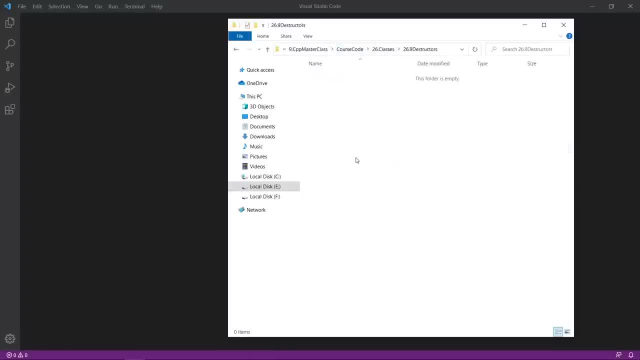 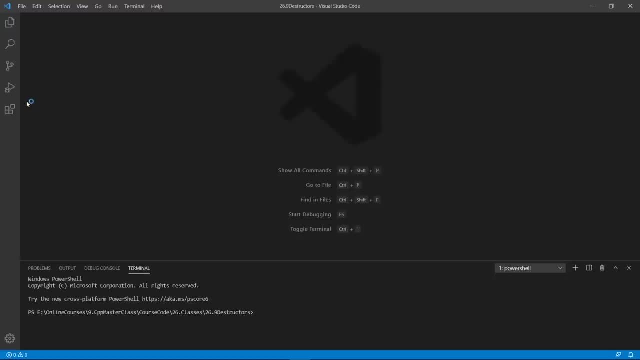 template files pretty quick and we're going to put them in place and after that we're going to open our folder in Visual Studio code by dragging and dropping here. this is going to open our folder and we will see our main cpp file here. we can open it and a cleanup and remove what we don't. 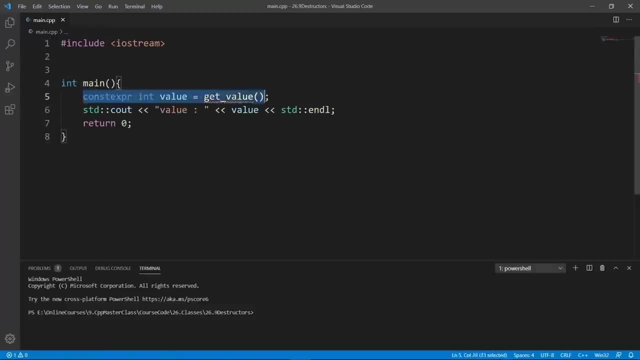 need. we have an unneeded breakpoint here. we can remove that and we're going to clean up the main function. the first thing we want to do is to put in our dog class. I am going to just put this in here because I don't want you to watch me type all this. that's just going to waste your time we have. 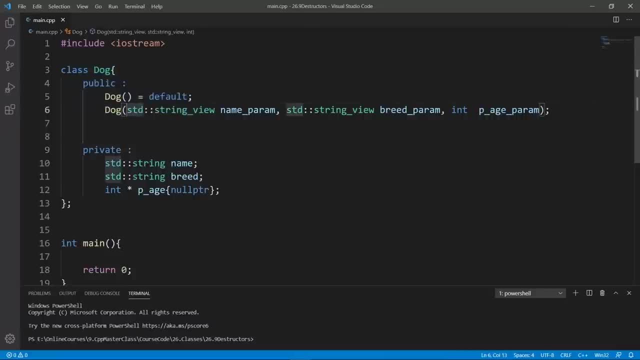 two sections in the dog class. we have a public section which is going to now contain our constructors, and we have a private section which is going to contain three member variables. we have two strings, one for the name and the other for the breed of our dog, and we have another one. 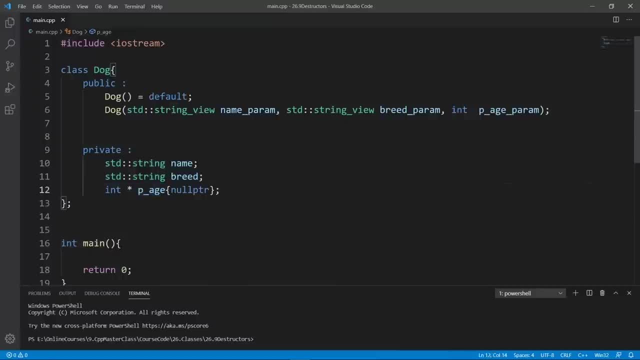 which is an int pointer which is going to enter the age of the dog, and you see that this is initialized to null pointer. one thing you should notice is that for our parameter taken constructor, we are passing the string information here using string views to avoid copies with the std string view type. you already know this because we learned. 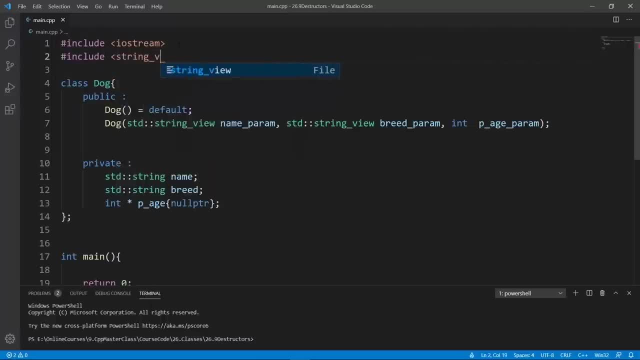 about this. but for this to work, we will need to include a string view. so let's do that. and now we have our class and we can use it however we want. so but before we do, we need to put in the implementations for these functions. one way we can do that is do that. 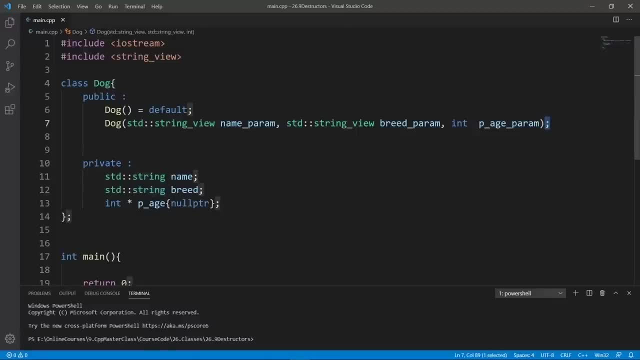 directly in the function here, but I want you to see that you can also do that directly outside of the class here. I don't think I have shown you this, but it is possible to do that. so we're going to grab the prototype for our constructor and say the scope resolution operator, and we're going to 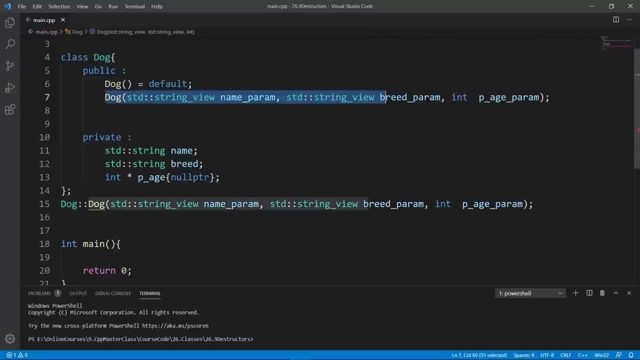 just paste in what we have copied, which is the prototype here, and we're going to go inside, put in the body. we're going to initialize these three guys. so the name is going to be initialized to name param and the breed is going to be initialized to breed param. we can do that and the age is going to. 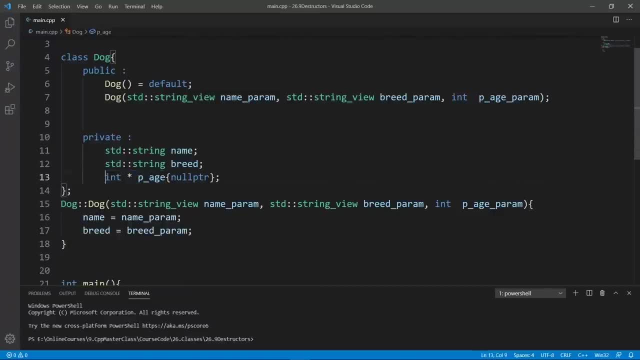 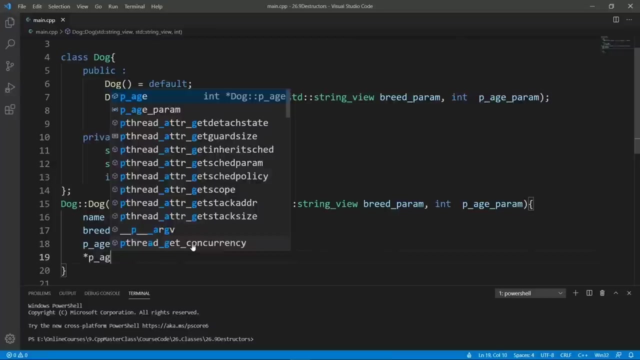 be dynamically allocated from the heap. you see that it is a pointer. so we're going to say ph equals new ant, because we're going to allocate dynamic space to store an end and we're going to put data in using our good old so the reference operator. we're going to say ph equals whatever ph parameter they passed and I 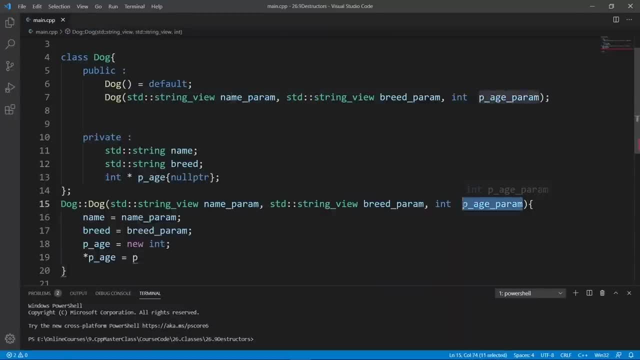 think we should say edge here, because it's not a pointer, so we're going to say age. I think this is going to do better. age param. this is probably going to be better and we're going to say age param. okay, so now we have our constructor in and it's going to allocate memory from the heap and 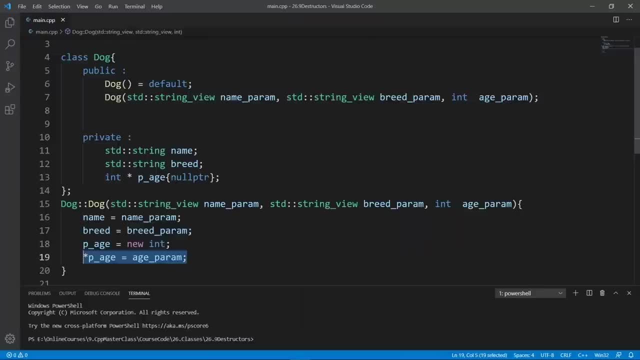 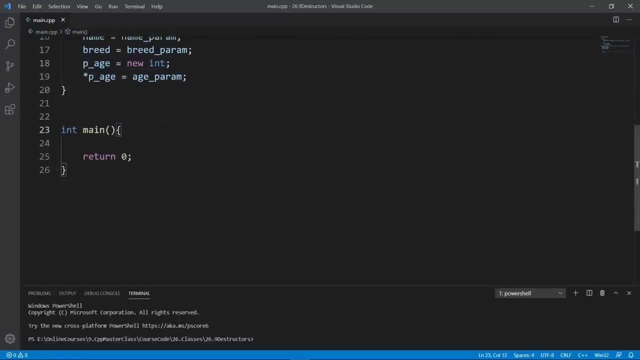 we're going to put data in that new memory location that has just been allocated to our class here. so this is our class and we can go in the main function and really use it however we want. for example, we can set up a dog object. so we're going to say my dog and we're going to give. 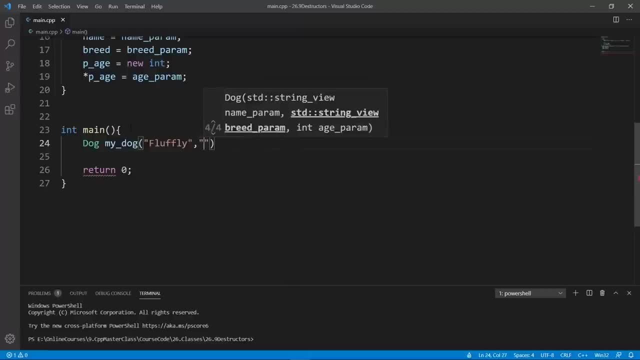 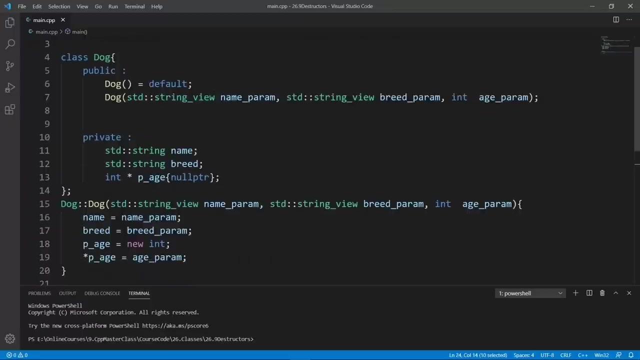 it a name. the name is going to be fluffy and we're going to put the breed in and it's going to just be a shepherd and we're going to put in the age, which is going to be, for example, a two. let's say our dog is two years old. this is a valid C++ code. it's going to be setting up an object of. 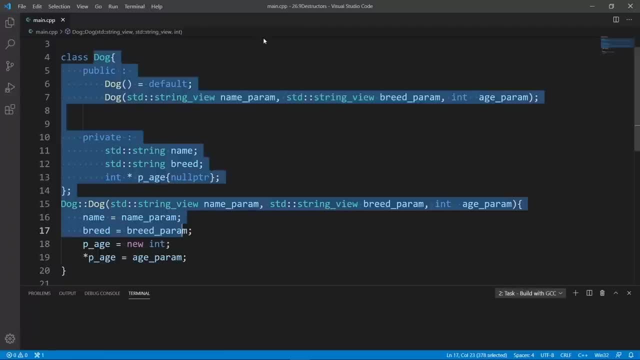 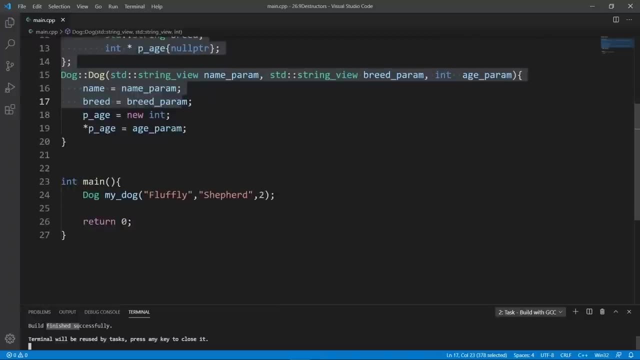 our class here and we can world to see that this program is going to world without a problem. so both is good. but if we run the program we're not going to see anything. but we don't really need to see our constructor here called, because we already know about constructors what we want to learn. 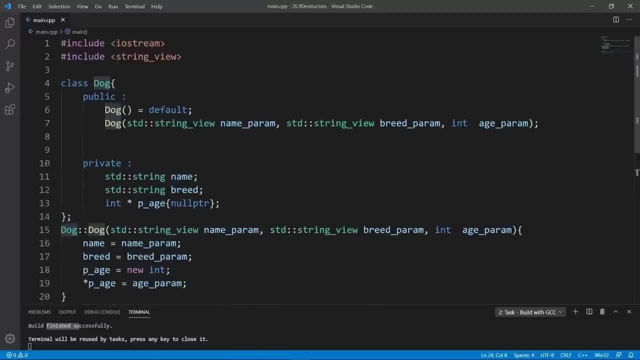 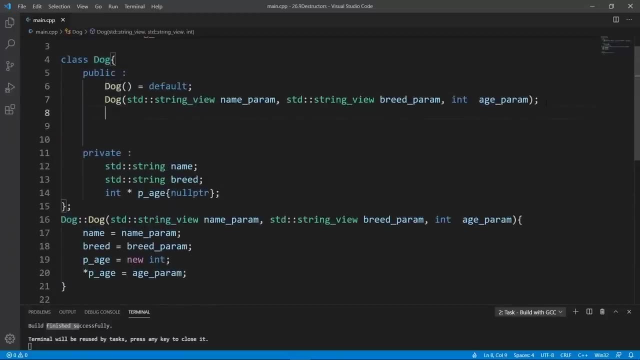 about are destructors, and these are special methods that are called by the compiler when your object dies. let's set up a destructor and see it called when our dog objects die. the syntax to do that is to use the tilde character. here you're going to say the name of the class you're going to put. 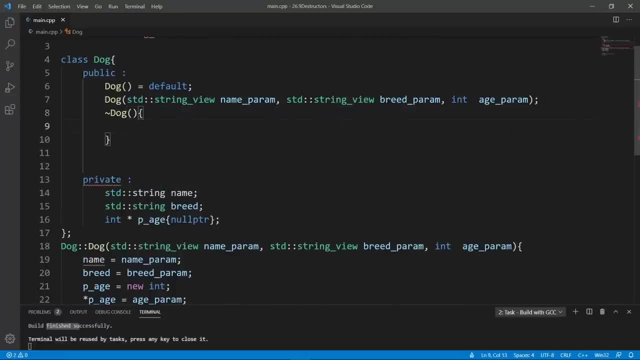 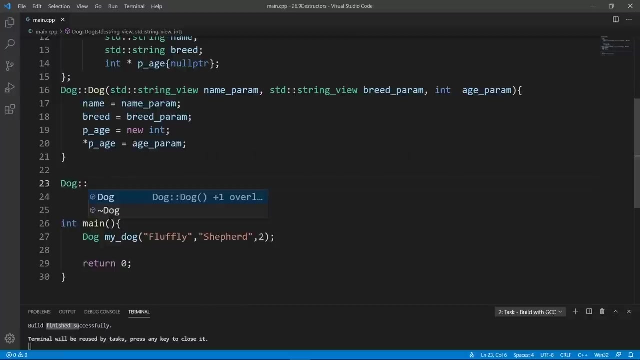 an empty parameter list and if you want, you can put a body and do whatever you want to do in the body of your destructor here. but again we're going to move the entire definition of the destructor to the outside. so let's go down and save that. we're going to say the scope resolution operator. we're 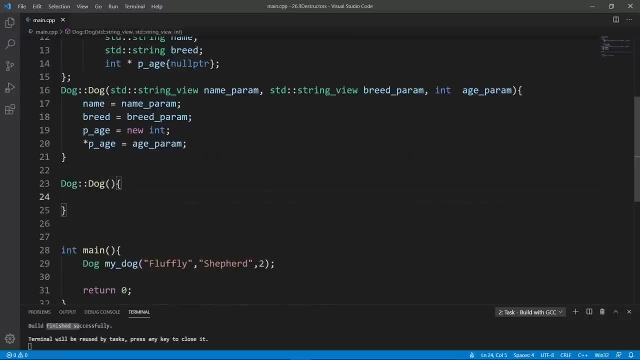 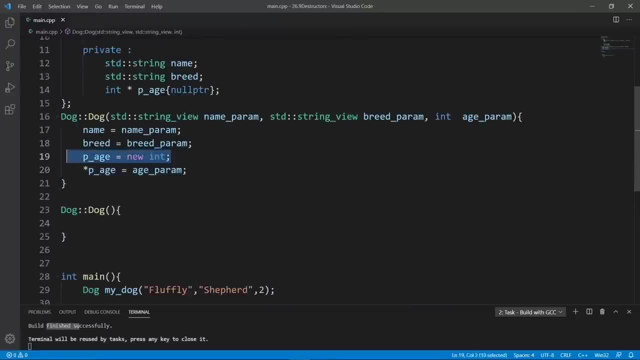 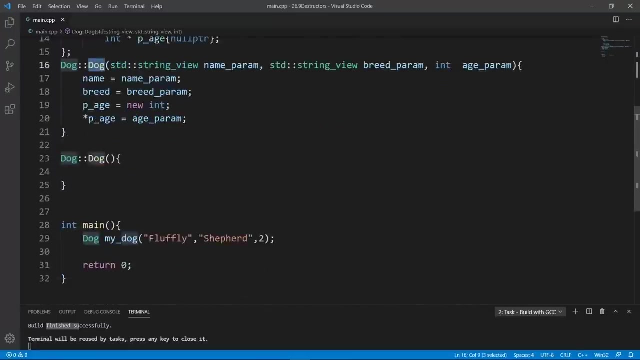 going to say dog and we're going to put in our body, and the first thing we want to do in our destructor is to release this memory that was dynamically allocated for us. if we don't release it when this dog object dies, we're going to leak memory and that's really bad. so let's do that. 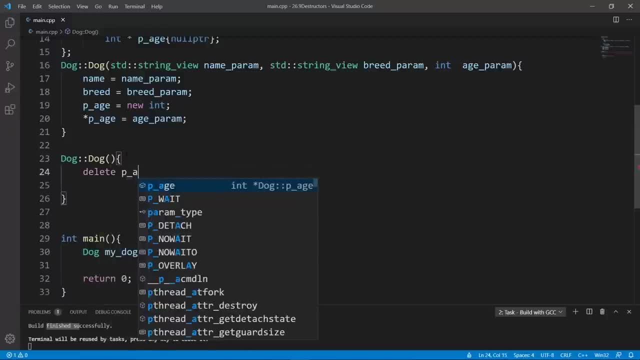 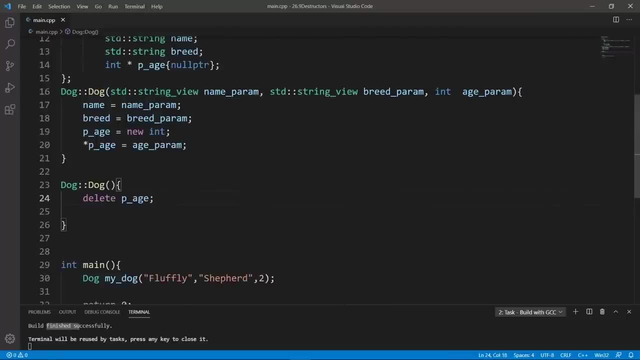 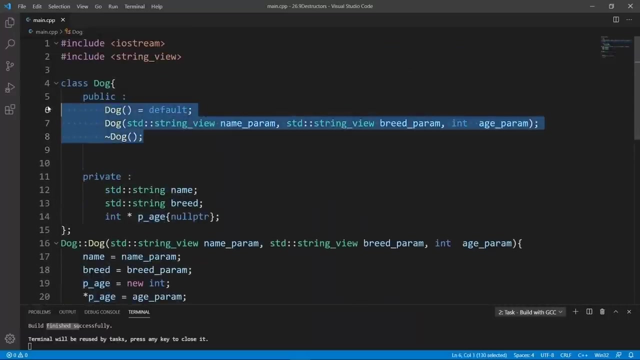 directly in the destructor. we can say delete and say ph. this is going to release the memory that was allocated in the constructor here and we have access to this ph variable because the destructor is part of our class. our function of your class is going to have access to any member variable, even if it happens to be. 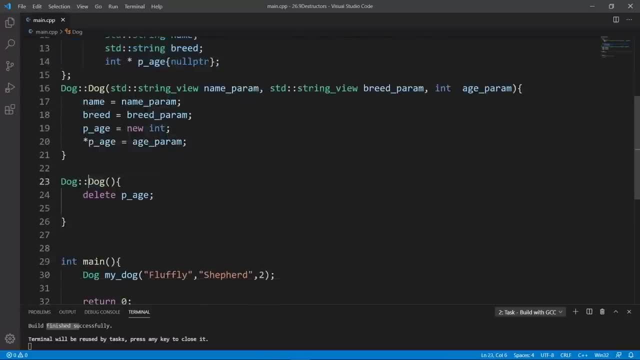 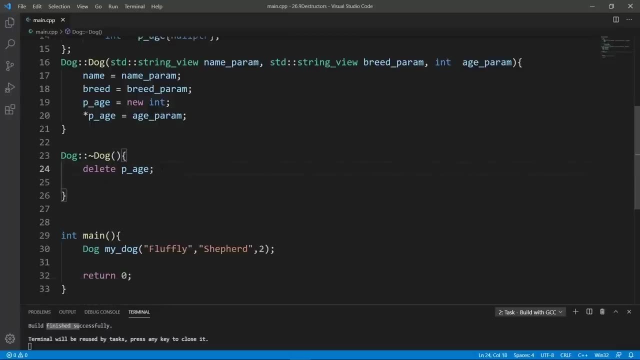 private. okay, so we forgot our tilde character. let's put that in here and this is going to be valid C++ code. but to really see things happening here, let's put in an stdc out statement. we're going to say dog destructor called for and we're going to say the name of the dog. let's say name. 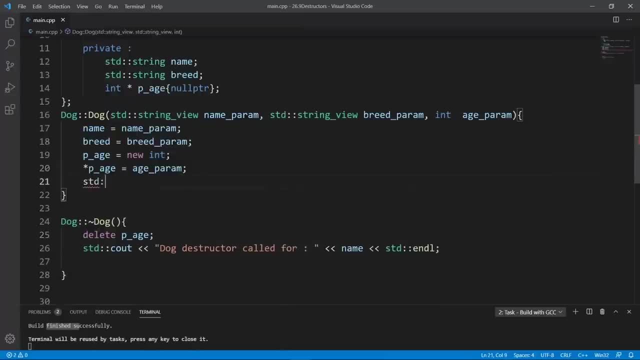 and we're going to say the same thing in the constructor. we're going to say stdc out and say dog, constructor called for, and we're going to say the dog name, we're going to use our member variable and now we have our thing in place. we have the destructor declared in the 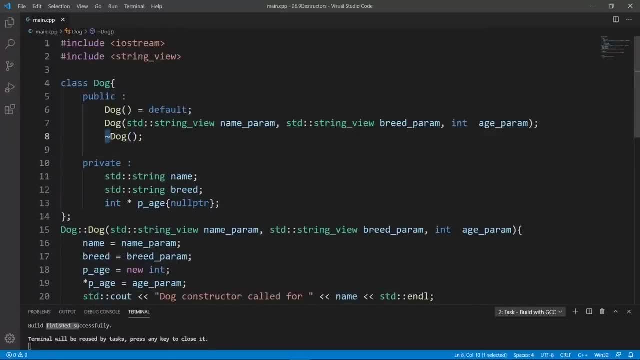 class definition and this is the syntax. again, this is what we really want to learn about in this lecture. we have the tilde character, we have the class name and we put an empty parameter list. let me tell you that it is not possible to pass parameters to your destructor. if you do that, you're. 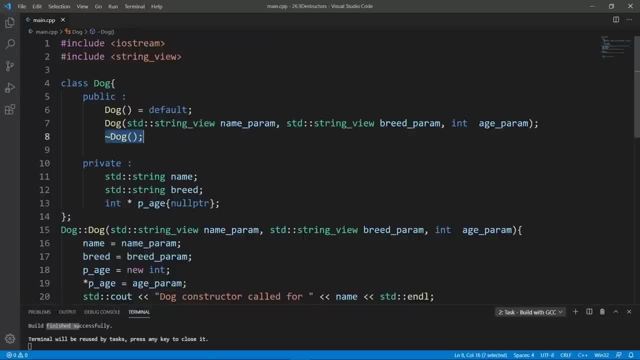 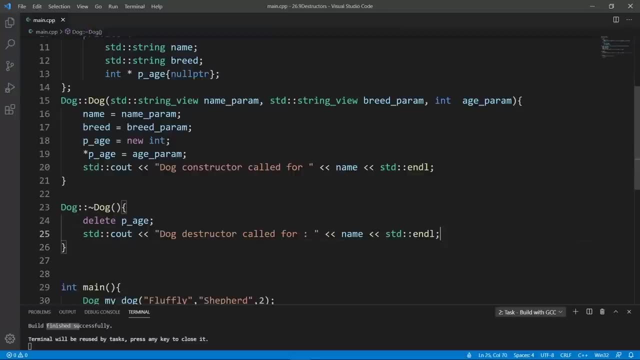 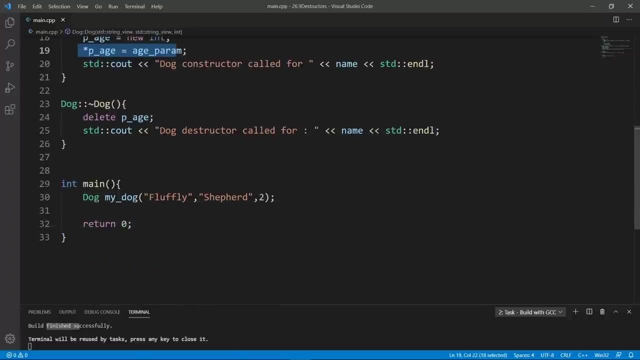 going to get a compiler error. destructors will always have no parameters in C++. here we have the definition of our destructor and it is going to release whatever memory we have dynamically allocated from the constructor. here, if we run this program, we're going to see our constructor. 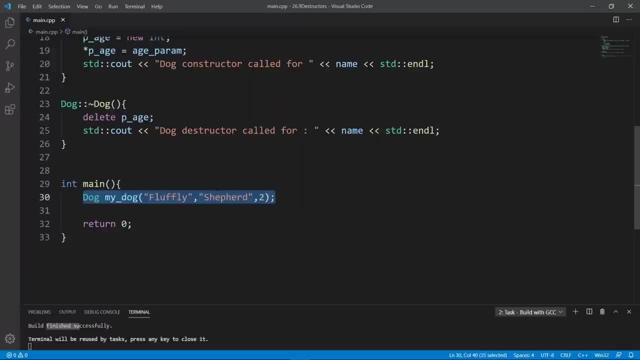 called as a result of this line here because we are constructing a dog object and we're going to see the destructor called when the main function is about to end. let's put an stdc out state to mention the main function here and say done just to prove that we have hit the. 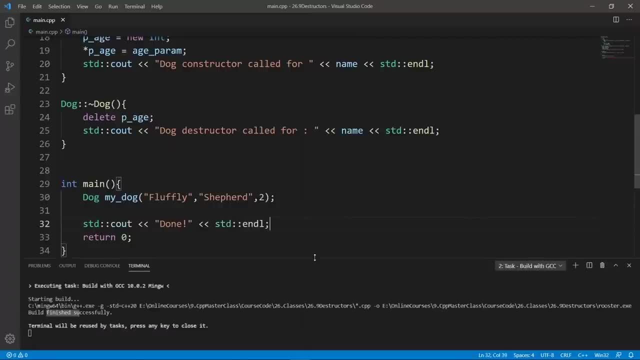 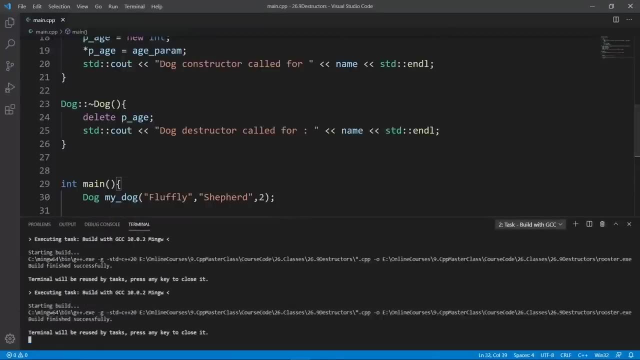 end of our main function here. I think this is useful and we're going to build, so let's do that. we're going to build with gcc. you're going to see that the build is good so we can clear and run our program. let's hit enter here and clear and run rooster. you're going to see that the constructor 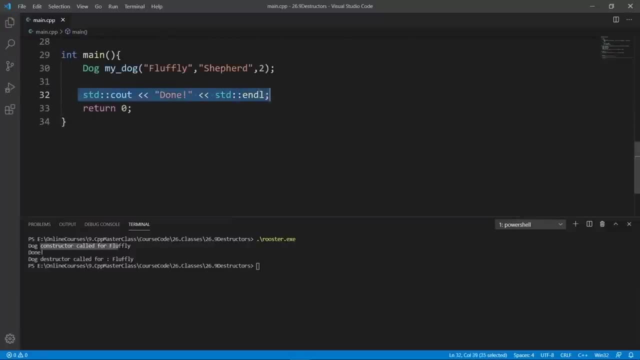 was called. we are going to say done when the main function is about to end, but before the main function ends we're going to destroy any stack data that we have in the main function and our dog object is on the stack, so it's going to be destroyed as part of that process and the destructor for a 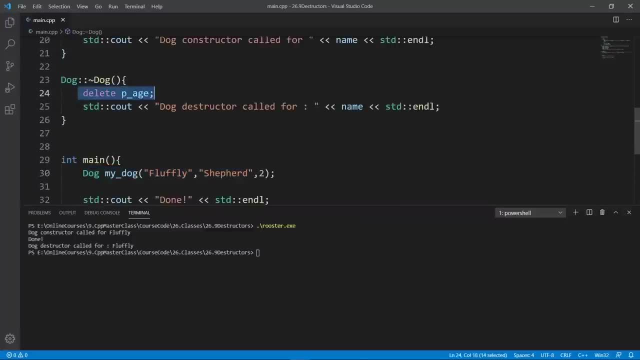 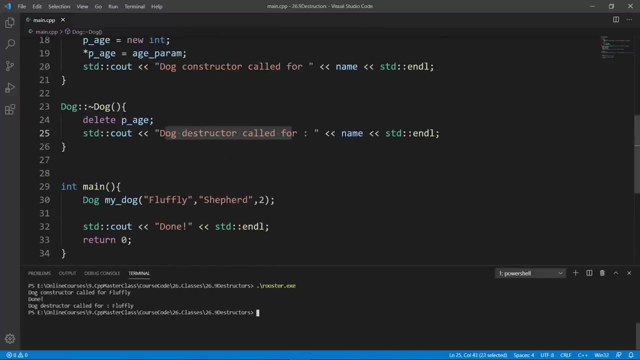 dog is going to be called and we're going to release our memory and we're going to say that dog destructor was called for whatever name we have assigned to our dog here. so this is how destructors are called when your objects are killed and we didn't. 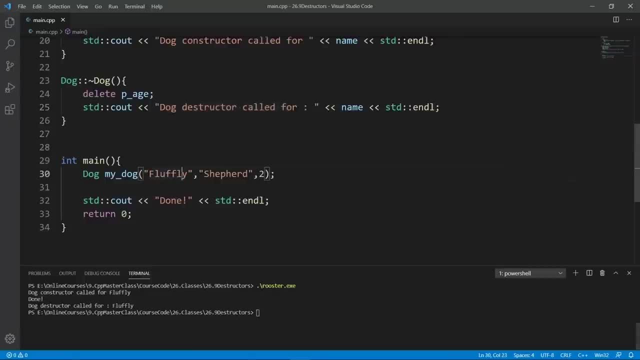 put in the correct name. we saved fluffily- let's say fluffy because that's what I wanted- and now you see that our destructor is really being called and releasing memory however we want. but we can also go a little further and show you another example of a case where destructors are. 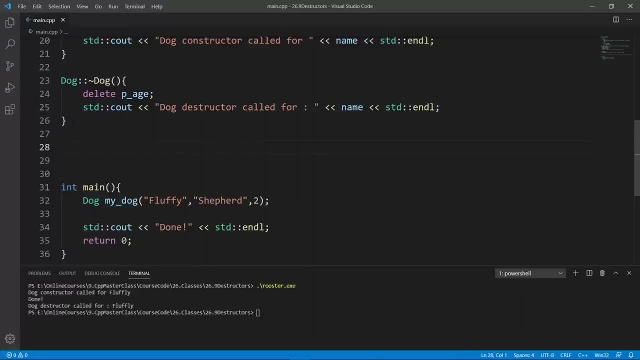 called and we're going to look at a function that sets up a local object of a dog. we're going to see the dog constructed and we're going to see it destroyed when the function is about to end. let's say, void some funk and it's going to be just some function to play with us. we're going to move our 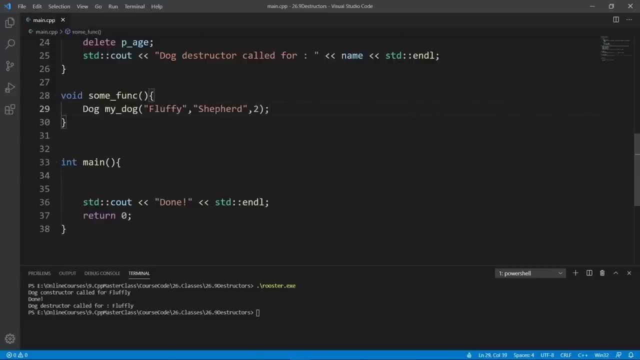 dog declaration and some funk here, and this is really it. we're going to call this function and when we call it, we're going to construct the object here. when the function is about to end, the compiler is going to call the destructor because it's going to destroy this object here and we're 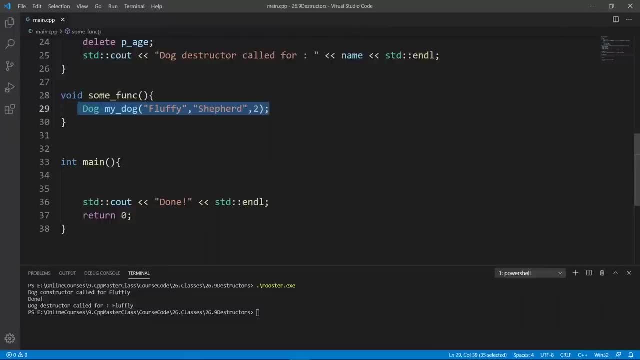 going to see the destructor called by that point, the some funk function is going to be popped off the stack. we're going to hit the main function here and we're going to say done and the program is going to end. let's call some funk in main here. so we're going to say some funk and we're going to 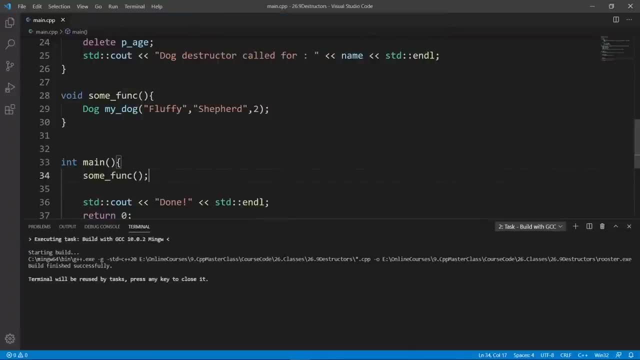 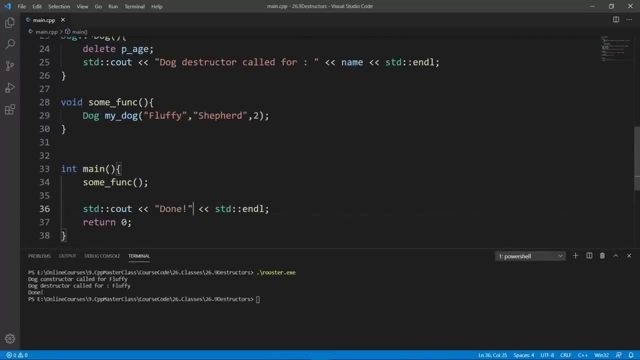 world to really see this happening. so we have both successfully. we cannot clear, clear properly and run rooster. we're going to see constructor called for fluffy, destructor called for fluffy and you see done. we have hit the main function and really finished executing our program. here we can even 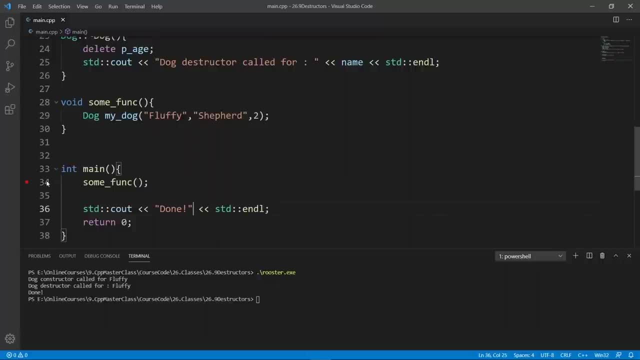 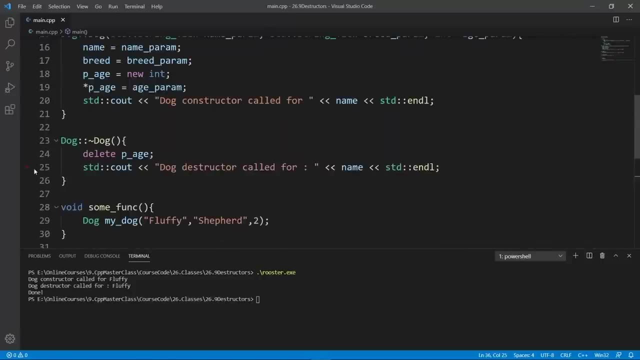 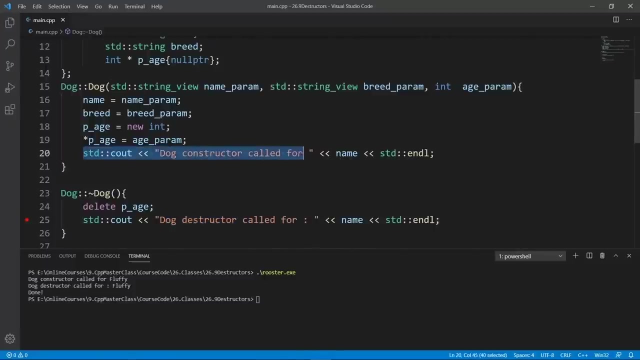 further, we're going to set up three break points: one in the main function here before we call the some funk function. we're going to set up another one in our destructor before we print the message here, and we're going to put another one in the constructor when we are about to print this. 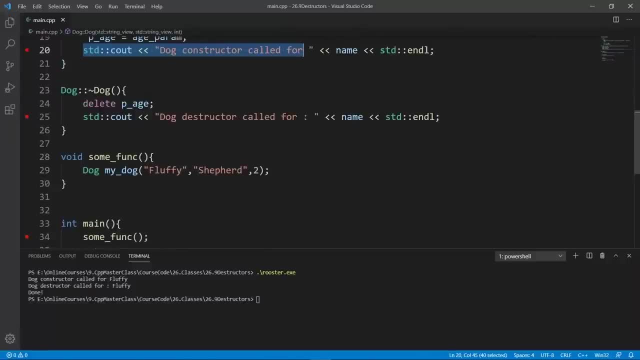 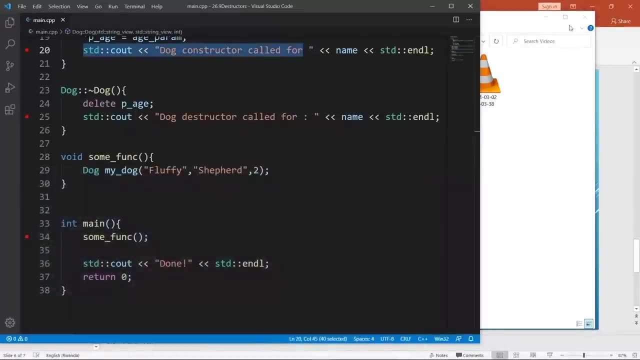 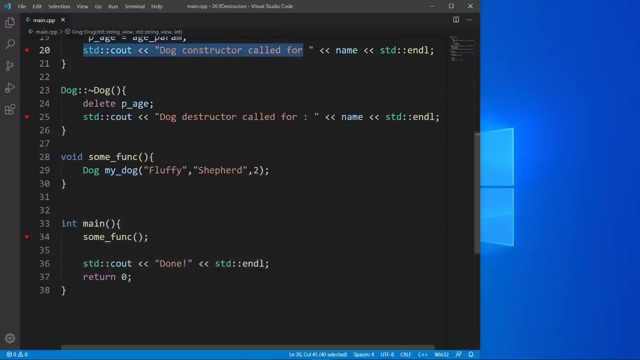 message here on line 20.. after we set up these break points, we cannot kill the terminal here and minimize a little bit. let's kill all these things here so that we have a clean. ah, we have a lot of windows here. okay, we have our editor here and now, if we go to 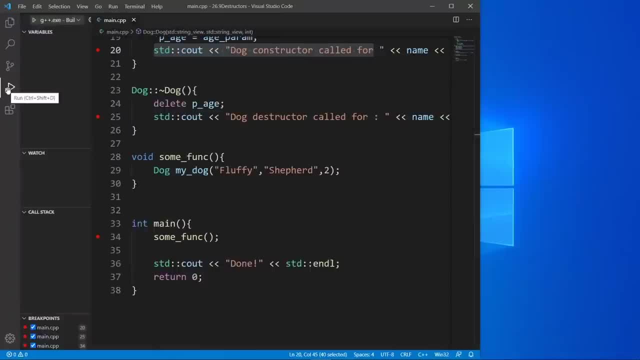 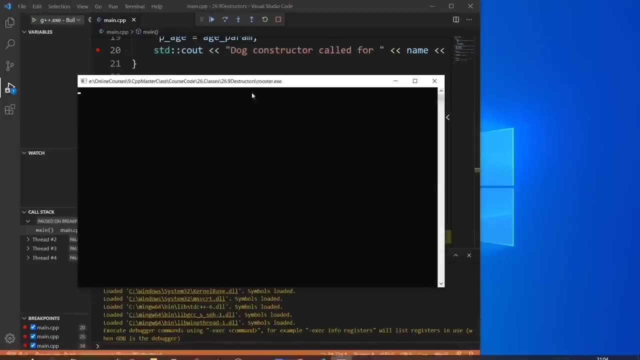 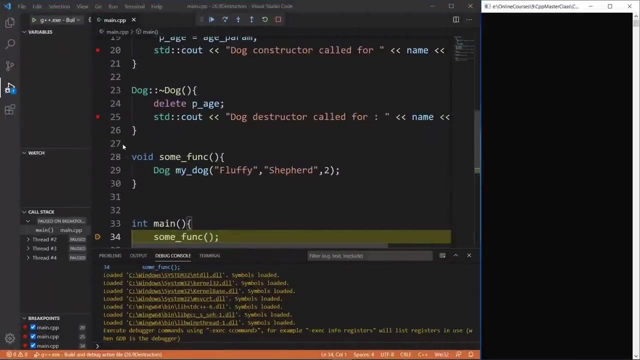 the tab here that says start or run. we're going to be able to click the green button here to start our debugging session. we are going to have our terminal here, so let's bring that to the side so that we can see things printed out nicely. let's do like this. and now we have hit the breakpoint in. 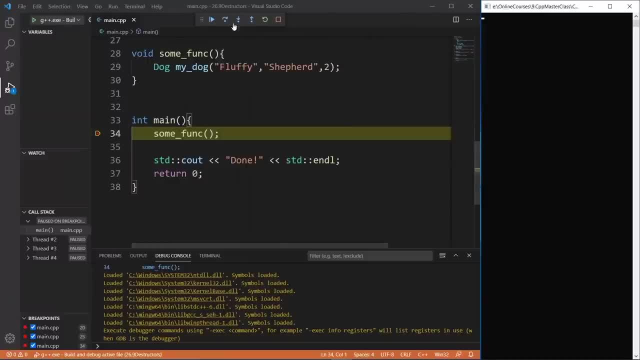 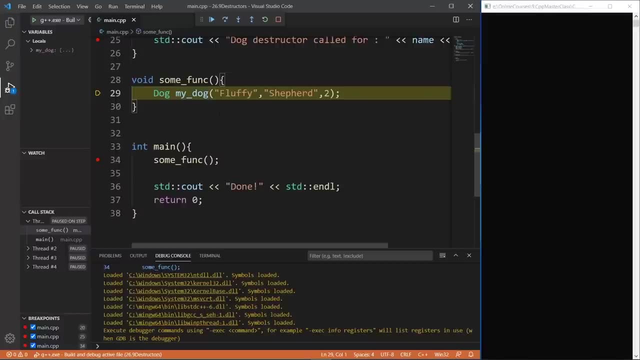 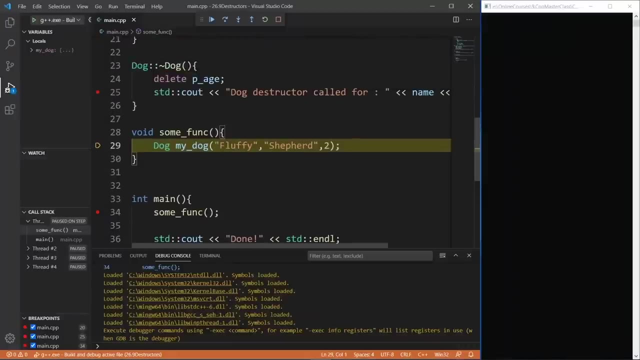 the main function. we can step into some funk function and we're going to do that using the step into button here. let's click that. we're going to jump into some funk. now we have the option to step into. but this is going to jump us into the logic of transforming the string literal here into a string view. because if you see the 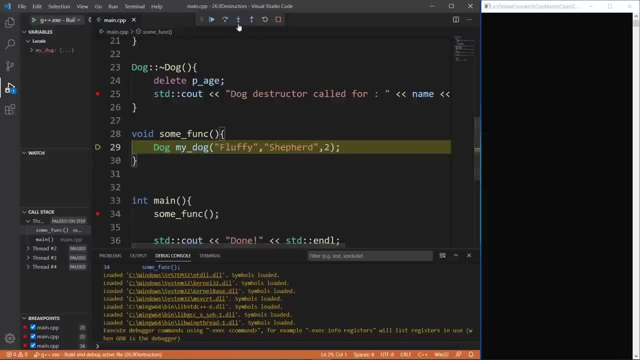 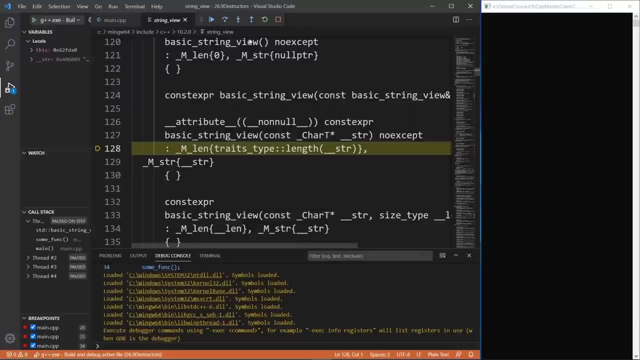 constructor is going to take string view parameters. we can actually see this. let's try and hit the step into button. you see that we are in the string view class and we don't really want this. so let's step out, and we're going to step over this so that we can. 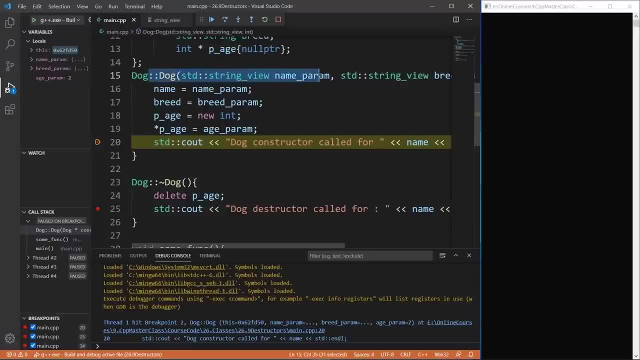 hit the next breakpoint and you see, the next breakpoint is in our constructor and this proves that the compiler is going to call our constructor here to build our object. if we step over this, we're going to print the message from the constructor and if we keep going, we're going to get out of. 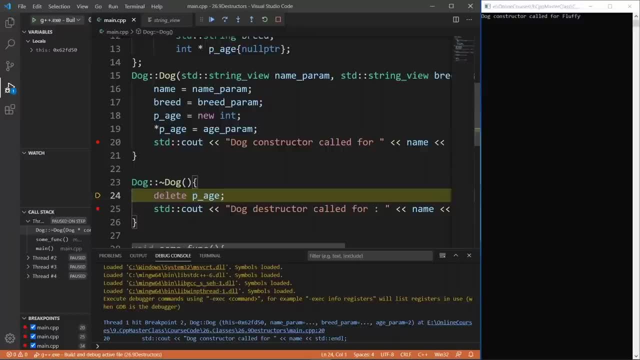 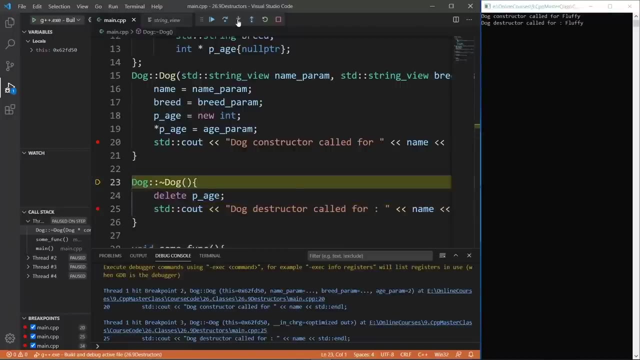 our constructor and you see where this is going to go. this is going to go in the destructor because before we leave the some funk function, our dad objects is going to be destroyed. so we're going to release our memory and we're going to print the message from our constructor and if we hit next and a step out of this, I think we can do. 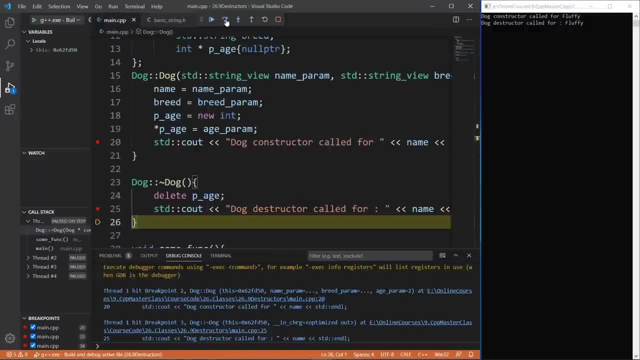 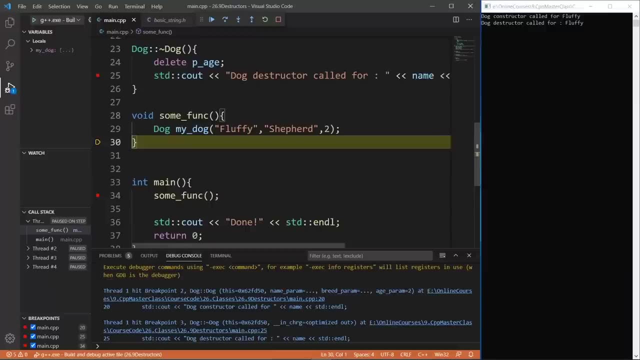 that, because this is logic we don't want. we're going to try and step over this. and now, if we hit next, we're going to come back in some funk, and some funk is already going to be finished. and if we hit next, we're going to come back in main and we're going to print done and the program. 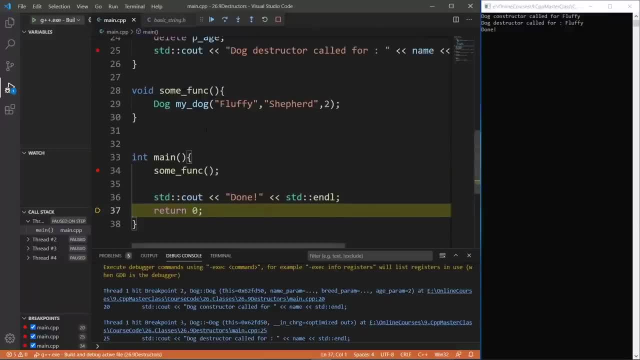 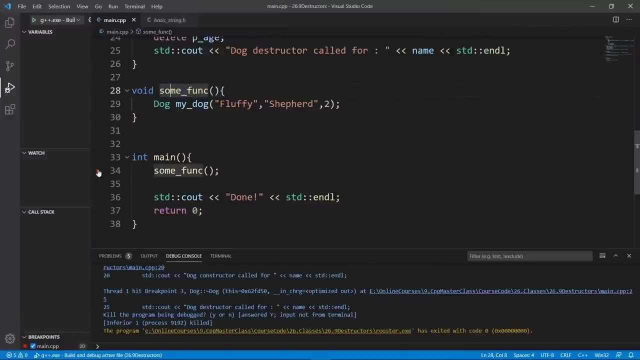 is basically going to be done. hopefully you can see that the compiler is going to call our destructor after it leaves some funk here, because it's going to be destroying the local object that we have inside- some funk here. so this is one case where the destructor is going to be called by the 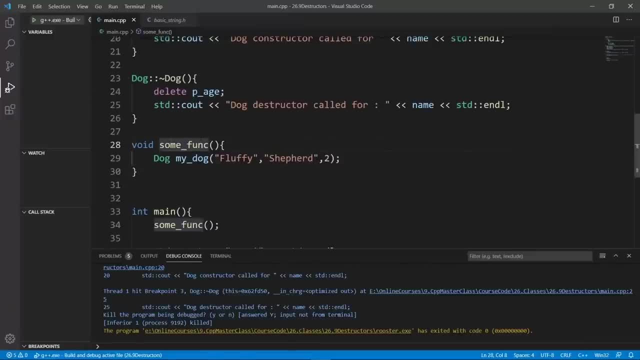 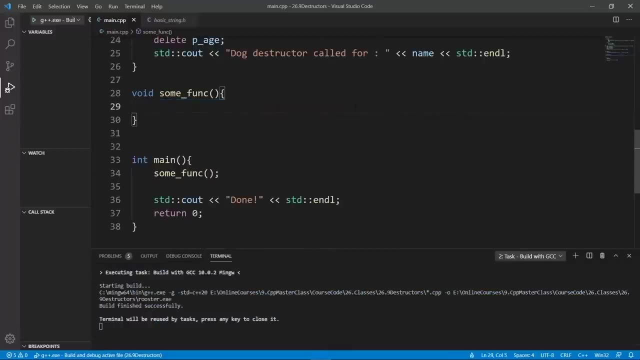 compiler, and it is. if you have a local object that needs to be destroyed, then function scope finishes. another case where the destructor may be called is if you pass a class object parameter by value. so let's change some funk here and make it take something by value. 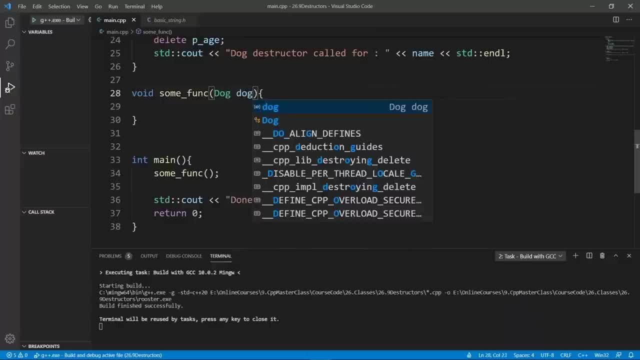 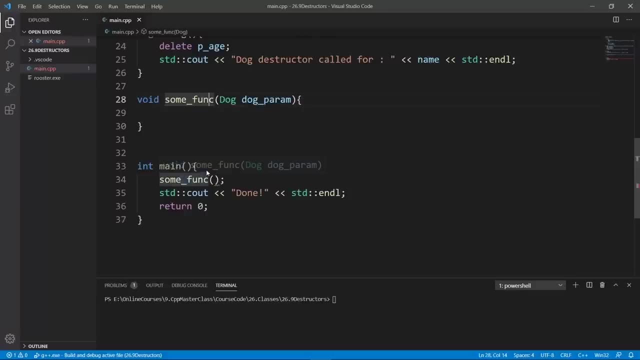 so we're going to pass a dog inside and we're going to say, dog, param, this is going to do. okay, now that we have changed some funk here, we can really do all kinds of crazy things with it. for example, we can set up our dog object inside our 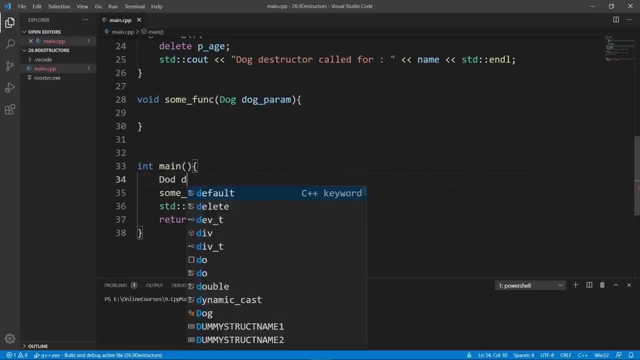 main function here. so let's do that. we can say dog and dog, the variable name is going to be dog. we can give it a name which is going to be fluffy, it's going to have a breed of Shephard, and we can give it the age of two, like we have been doing all along. we can call our function with the dog. 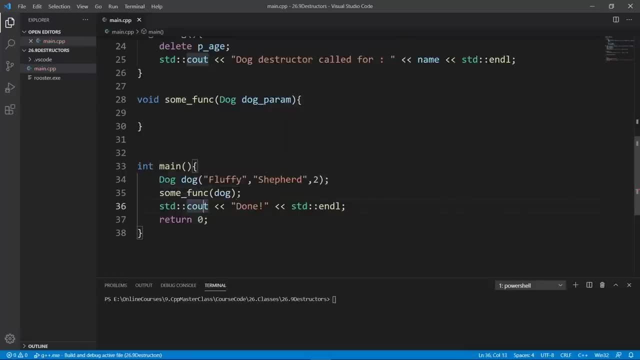 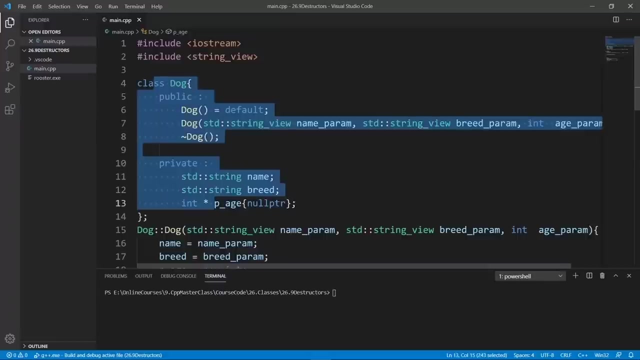 object here. but be careful about what is going to happen here. when we do something like this, we're going to be passing by value and the compiler is going to see that it needs to copy a dog object. now we haven't really told our class here how to copy dog objects and we do that through. 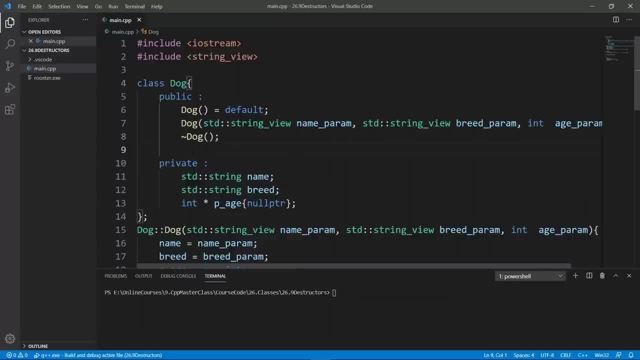 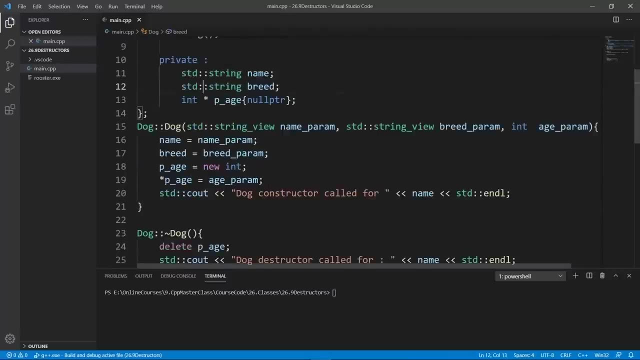 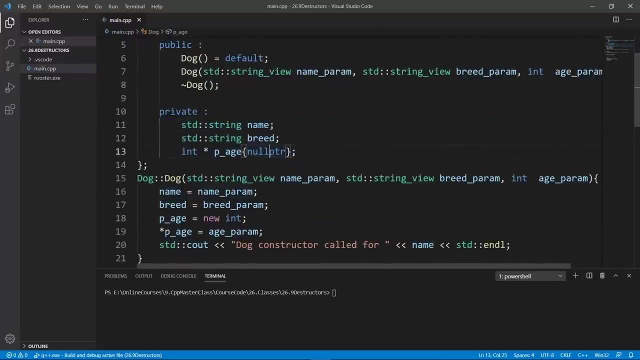 constructors we call copy constructors. we haven't really learned about yet, but what the compiler is going to do by default is copy these things member by member. so it's going to set up a dog copy object which is going to be initialized with empty strings and a null pointer here, and then it's. 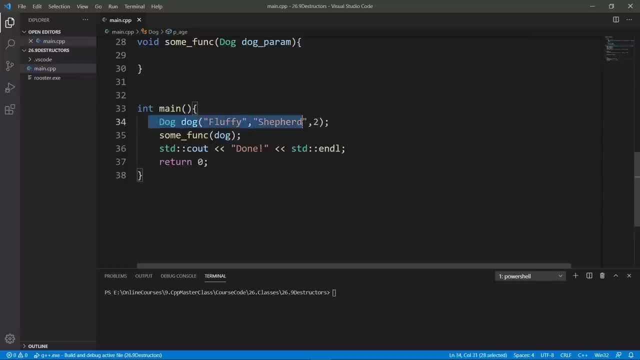 going to copy from our dog object that we have here. it's going to take the name and copy that in the name and member variable of our dog copy. it's going to take the breed and copy that n in the second member variable here and it's going to take the age from our dog and copy that n. the problem is going to come to this pointer. 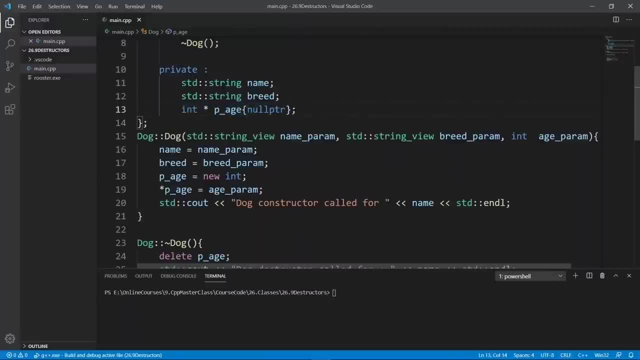 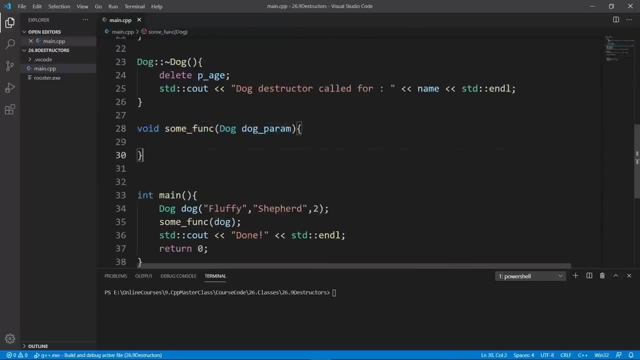 here. it's going to copy the address and it's not going to copy what is pointed to, and this is going to be a recipe for a disaster. I don't really want to go through this right now, but if we try to run this program, it's not going to work like we expect. for example, if we pass fluffy here, we're going to see things. 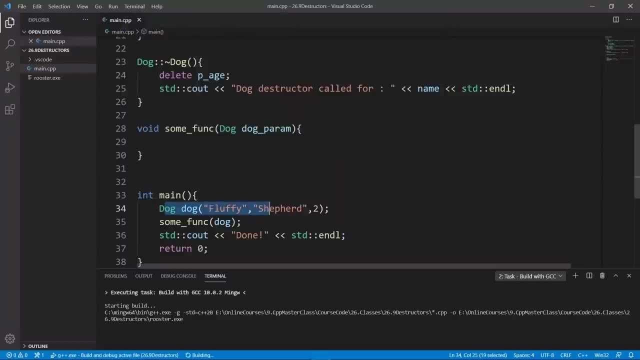 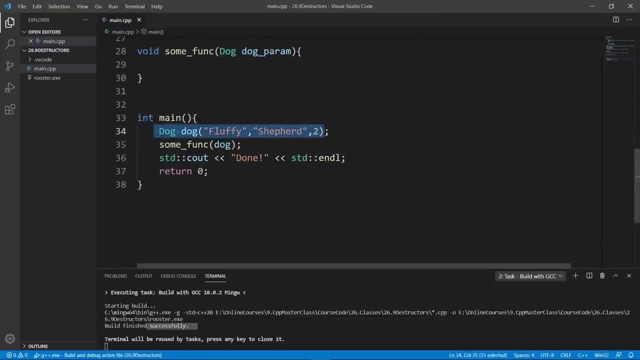 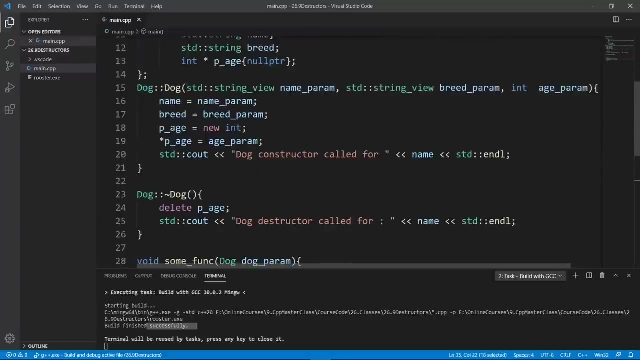 that we don't expect, so let's try to build. we're going to build with gcc and the build is good. so what we expect is to have the constructor of fluffy here called and we're going to copy the dot object for use in some funk here and to set up this copy. it's not this constructor here that 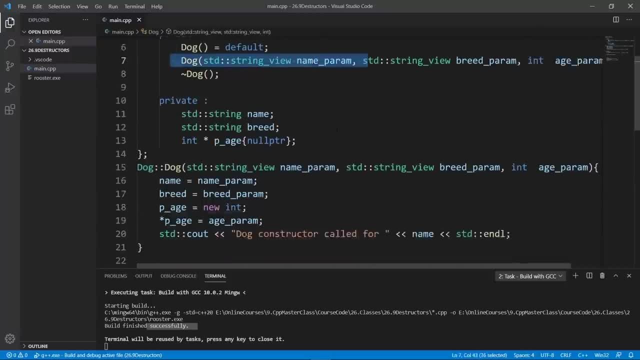 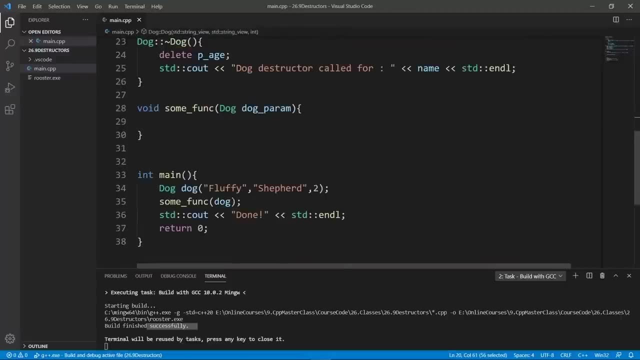 is going to be called, so it's not our constructor here which is going to be called, so we're not going to see this called for, the copy that we set up inside some funk. another thing is because now these two dog objects are pointing to the same. 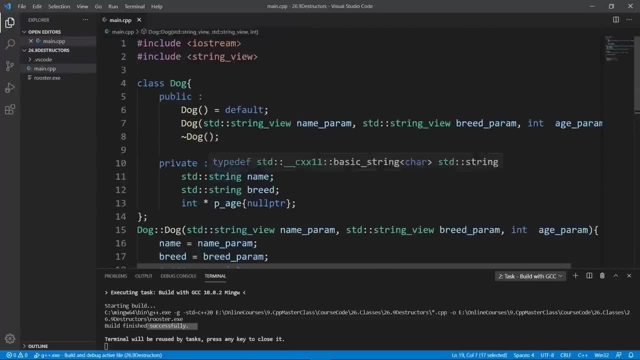 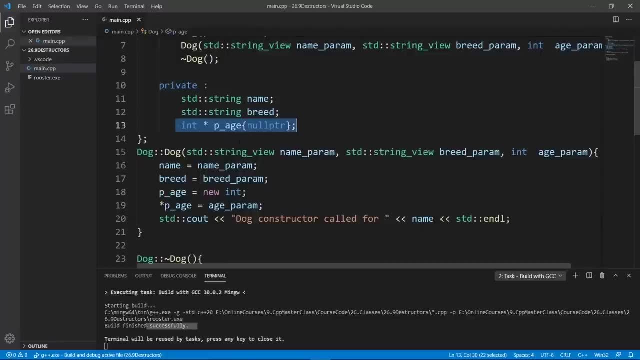 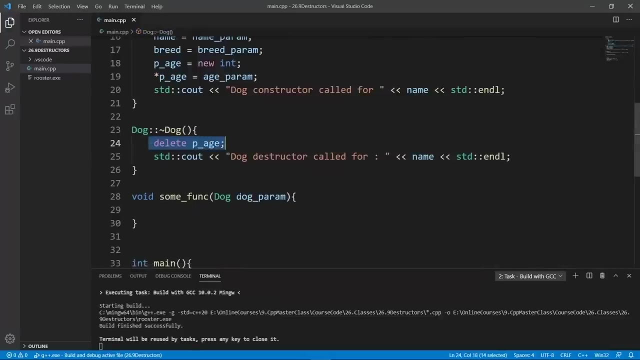 thing, because what we just copied is the address as we see in our member variable. here the two dog objects are going to be pointing to the same thing in memory and when we hit the destructor we're going to call delete twice, and this is going to be a recipe for a disaster. our application: 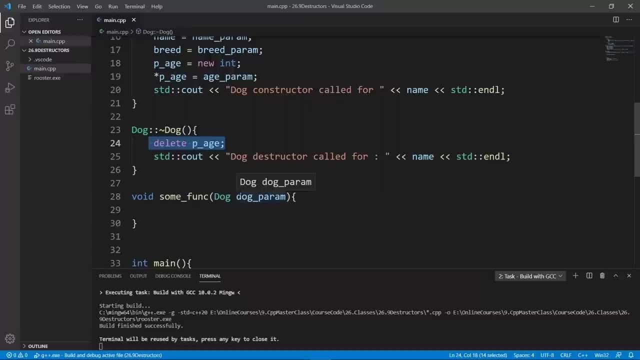 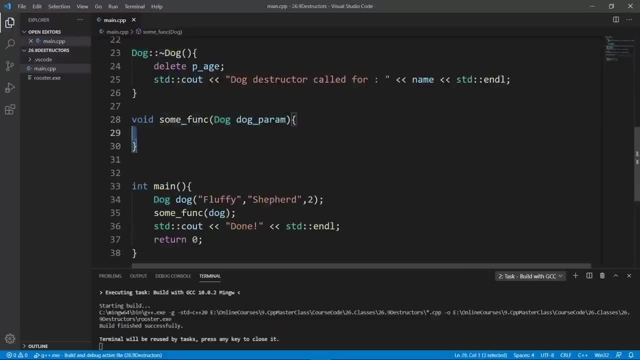 would really crash. you already know that deleting a pointer twice is really bad. we shouldn't do this. and we are doing this here because we are copying. I realize this is a slightly confusing example, but what I wanted to know is that if you pass a class object by a value like this, the copy you have. 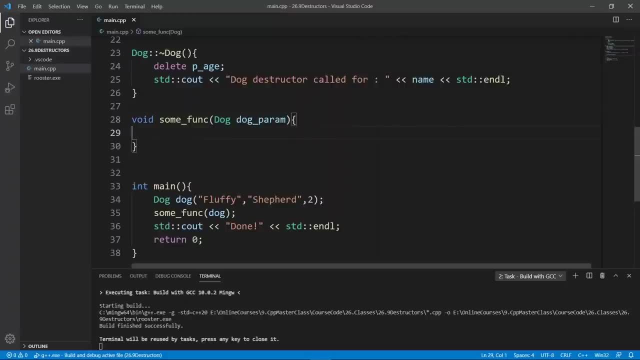 inside is going to cause for the destructor to be called when the function exits, because the copy is going to be scoped inside the function here. so let's take out this example because it really is confusing, but I hope you know that and I am going to show you that. another 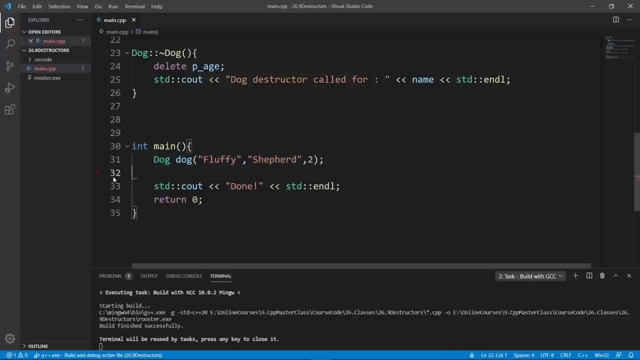 case where you might see the destructor called is when you call the destructor explicitly using the delete operator on your object, so we can set up some funk again. let's do that some funk and we're going to repurpose it. and this side we're going to set up a dog object, so let's grab this and reuse. 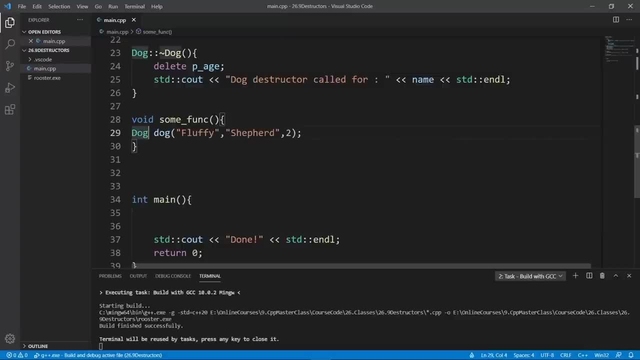 that in our function here and we're going to say dog pointer, so let's say dog pointer. we're going to say p dog, p underscore dog. it's going to be equals to new dog and we're going to pass in what we need to initialize our dog object with. this is going to create a dog object on the. 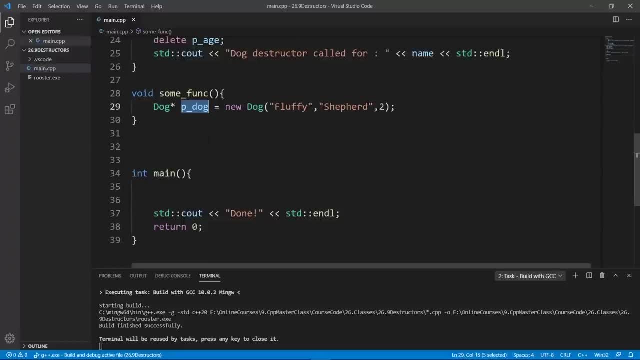 heap and it is going to be pointed to by p dog here now. I want you to see that if we don't explicitly release the memory that we allocate through the new operator, we're going to leak memory. so we created an object on the hip here, but 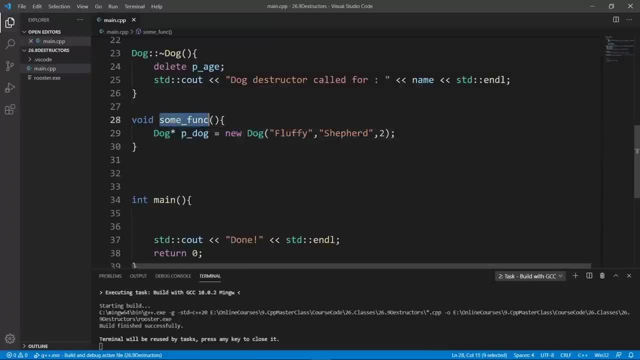 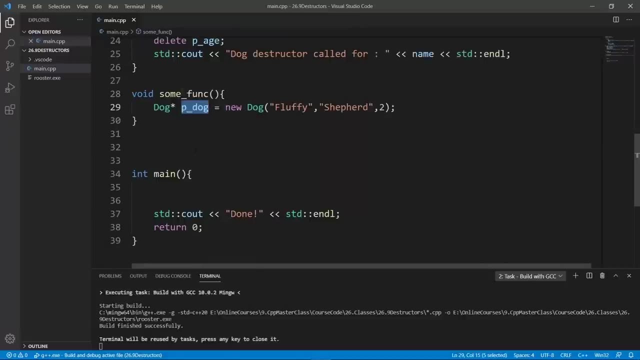 deleting that in some funk, when some funk exits, we're going to lose this pointer, this variable, because it is on the stack itself and we won't have any way to release this memory. let's call some funk here and really show you this. so we're going to call some funk and we're going to build. 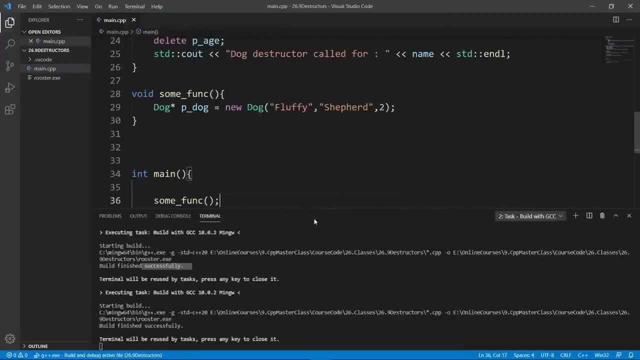 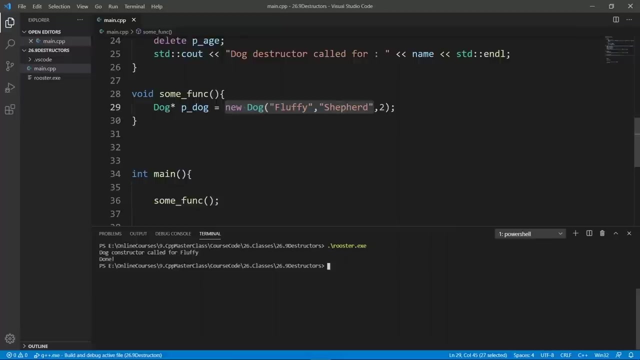 let's use gcc for that. the build is good. we can bring this up a little bit and clear and run rooster. we're going to see that the constructor for fluffy was called because of this new operator, but we didn't see the destructor called, and this is really bad. so for the destructor to be called, we need to explicitly. 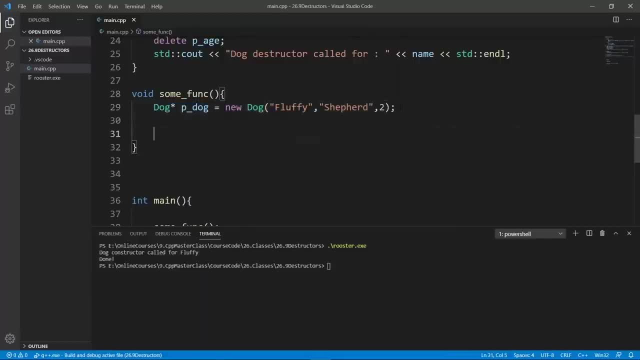 release the memory in this function here, and we do that by using the delete keyword and saying the pointer that is pointing to the memory that we want to release. if we do this, this is going to cause for the destructor of Doug to be called and if we run, we're going to see our destructor. 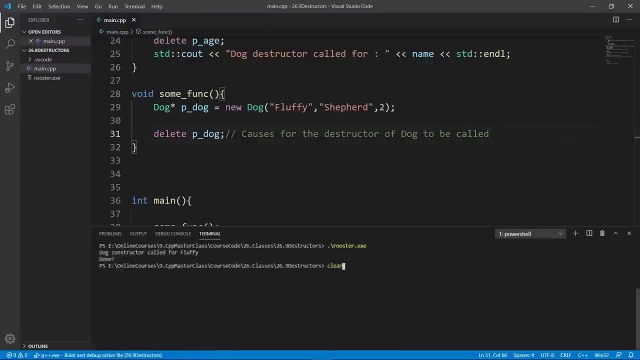 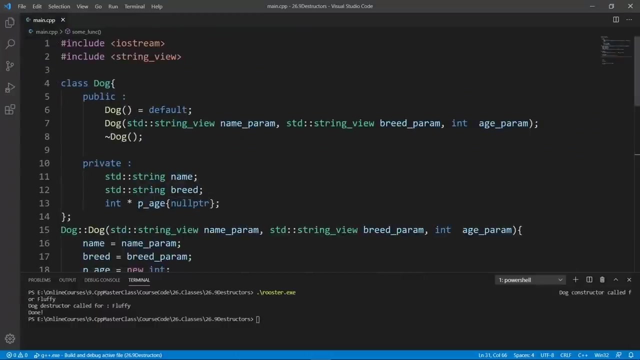 called. let's do that. we're going to use gcc. the build is good, you can clear and run rooster now that the constructor is called for fluffy and we have the destructor called. this is really all I wanted to share with you in this lecture. I apologize if you found it confusing, but if 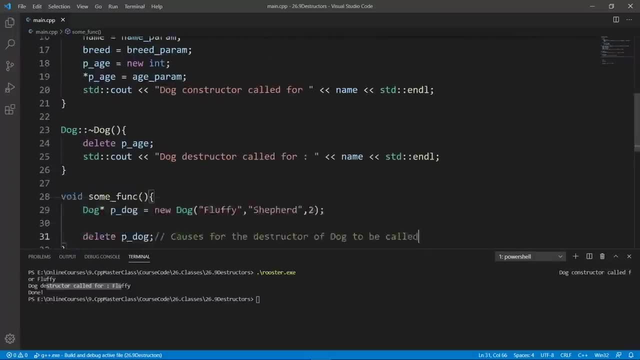 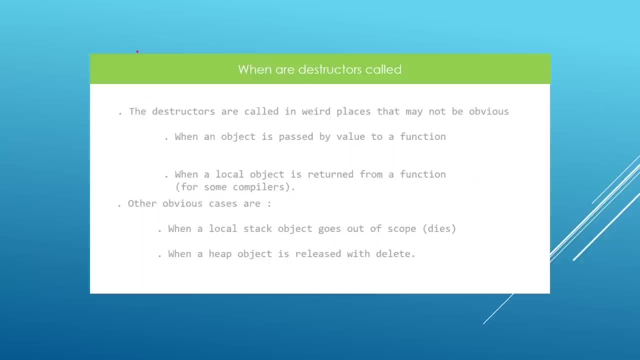 you have any problem, I am always available. please do ask and I will do the best I can to help you out. so the destructor is a special method which is going to be called when your object dies. it is going to be called when an object is passed by value to a function. we have seen an example that. 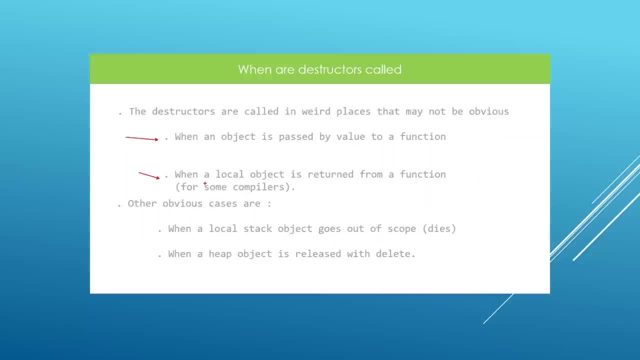 is going to be called when a local object is returned from a function by value. but this is going to be compiler dependent, because some compilers are going to optimize this out and make it look like when you returned by reference. so I don't want to go into this, because this is. 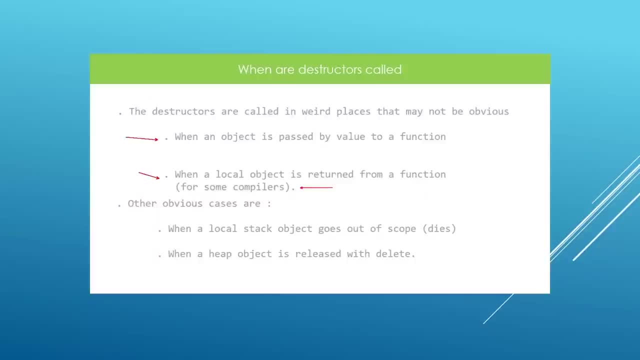 subject to compiler optimization. but other cases where you're going to have your destructor called is when a local stack object goes out of scope and when a heap object is deleted through the delete keyword. this is really all I had to share in this lecture. I hope you found it interesting. we are 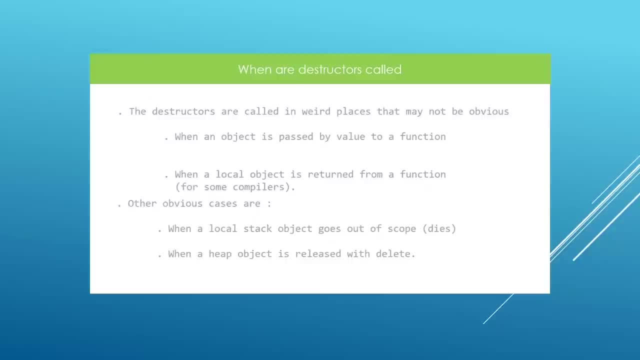 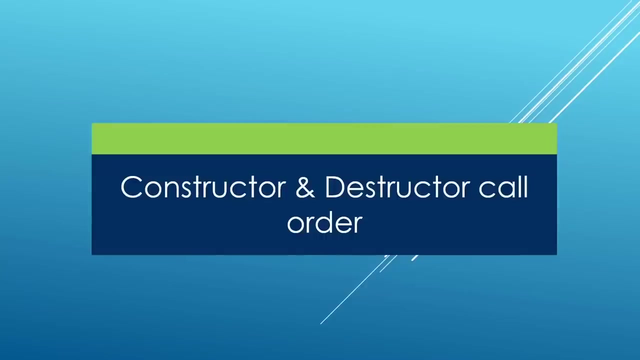 going to stop here. in this one and the next one, we're going to see the order in which constructors and destructors are called, and you really need to be aware of this. go ahead and finish up here and meet me there. in this lecture, I wanted to raise your awareness on the order in which. 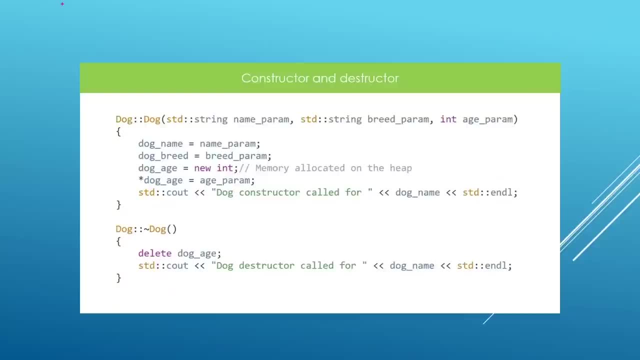 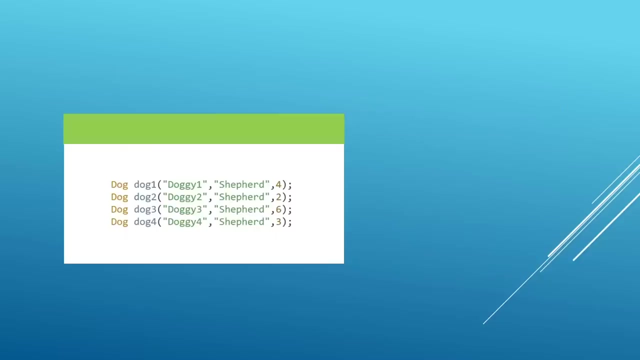 constructors and destructors are called. suppose we have our class, which is Doug, here, and we have the constructor which is doing its thing in the body, here, and we have the destructor which is releasing our memory and printing something out. so suppose we have created a few objects of this class here and they have different names and they have the same breed. 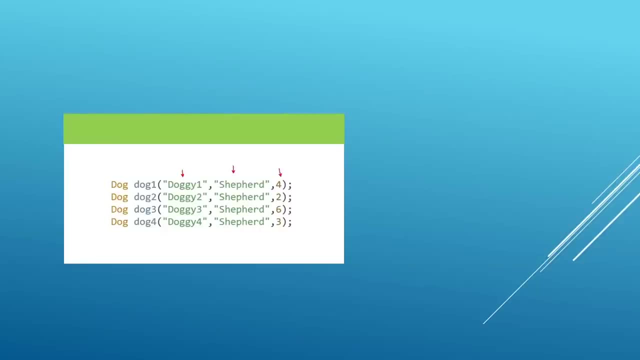 and different ages, as you see here. and if we run this code in main, what do you think we'll see printed from the constructors and the destructors? if you asked me- and I was learning about C++- I would say that the constructors are going to be called in order: Doug one, Doug two, Doug three, Doug four. they are going to be constructed in. 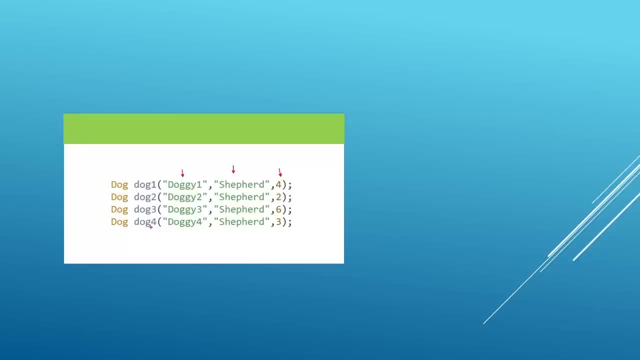 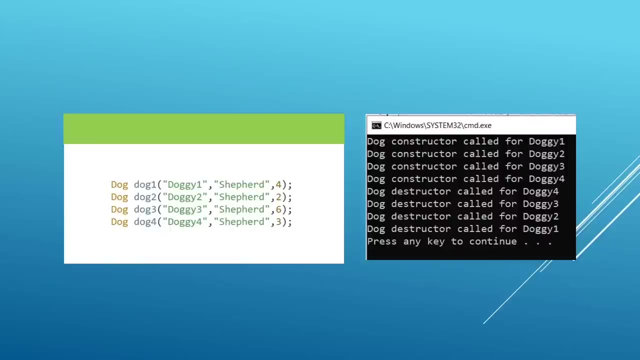 this order and the destructors would be called in the same order, but this is not true. the destructors are going to be called in the reverse order, as you see on the right here. so we're going to call this constructor for Dougie one, Dougie two, Dougie three, Dougie four, which is exactly what I expected. 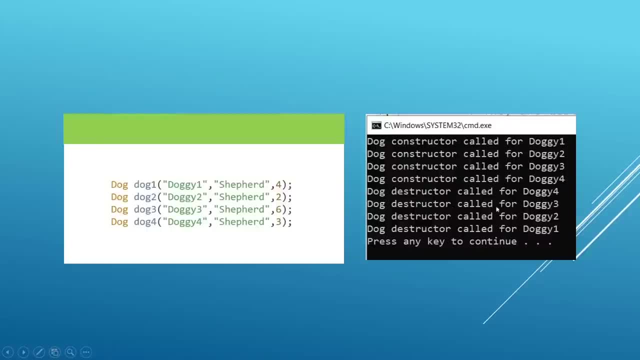 but you're going to see that the destructors are going to be called in reverse order, so the object that was constructed last is going to be destroyed first, as you see here, and the object that was constructed first is going to be destroyed last, and the compiler follows this order to make it. 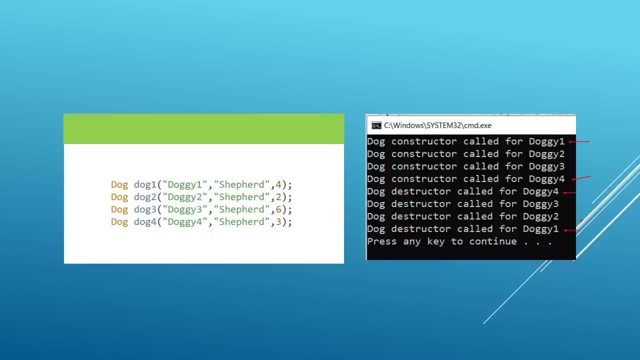 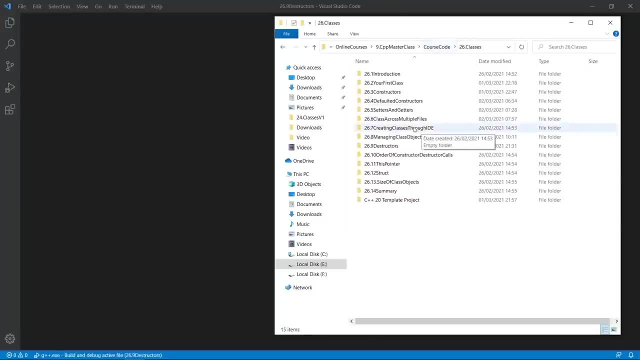 easy for it to do things. we can't really get into those details, but for now we're going to head over to our working folder. the current project is order of constructor and destructor calls. here we're going to grab our template project pretty quick and we're going to put them in place- the files I mean. 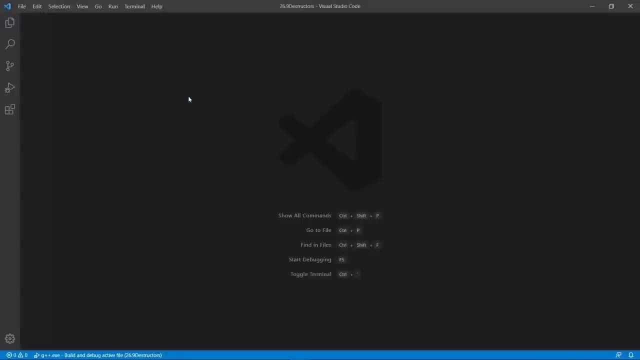 and we're going to open this in Visual Studio code, like we have been doing all along. this is going to open up our folder. we can close the left sidebar here and let's clean up our main function. we are going to bring in the class for Doug. 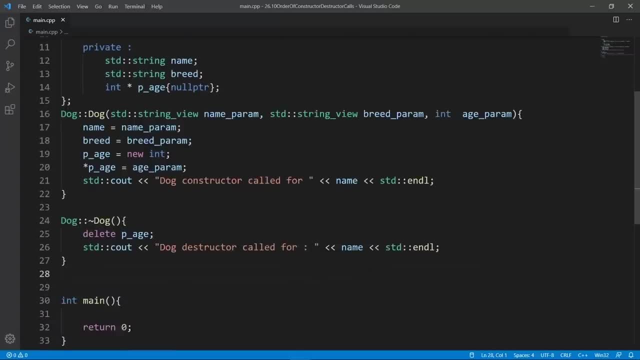 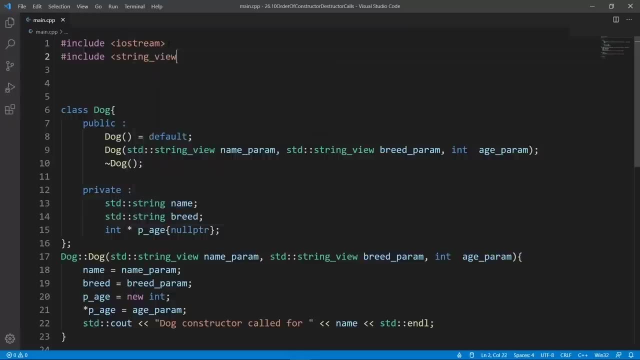 from the last lecture. this is exactly what we had there- no change- and we're going to include the string view library for this to work. so we're going to include string view here and once we do this, we're going to head over in the main function and set up a few objects of the dog. 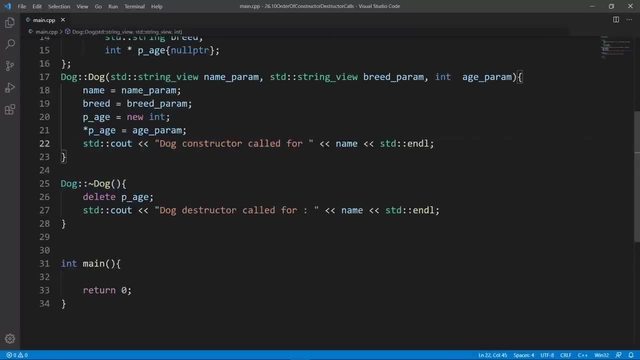 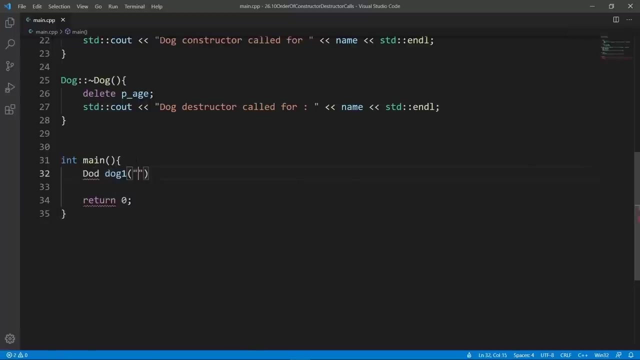 class here. but before we go there notice that we have a few stdc out statements in our constructor and destructor and we want to see the order in which they are called. so we're going to set up four objects of our dog. we're going to say dog, dog one, and we're going to say the name to be doggy one, and 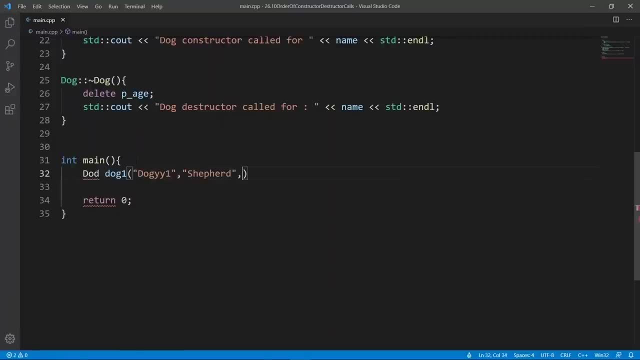 it's going to be a shepherd and it's going to be, for example, two years old. why not? we should say dog here, and we are going to copy these four times here and we're going to call this dog two, the other is going to be dog three and this is going to be dog four, and we're going to say the same thing. 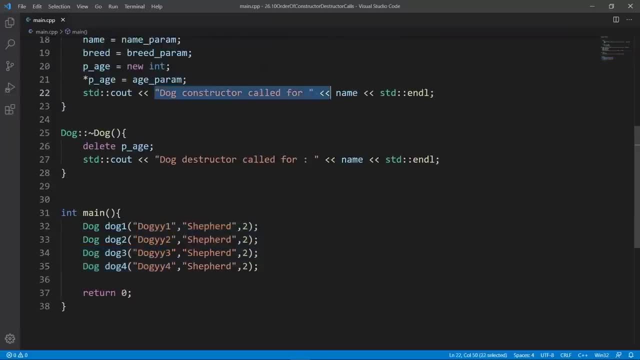 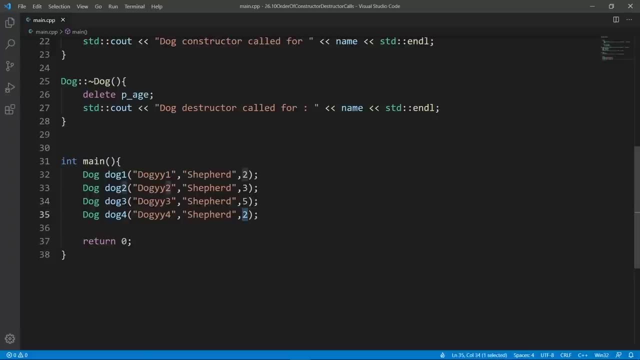 are what is really important, because we're going to see them printed out here. but if you want, you can change the ages. let's make this a three, let's make this a five, let's make this a one, why not for doggie four? and now we're going to run our program. if we run it, we're going to see the constructors. 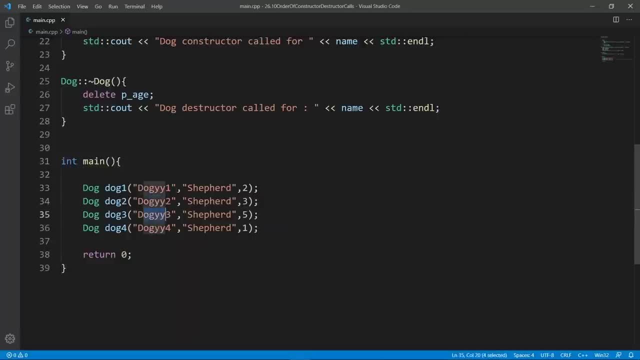 called in the order: doggie one, doggie two, doggie three, doggie four. and the destructors are going to be called in the reverse order: doggie four, all the way to doggie one. let's build and show you that this is actually the case. so the build is good. we can bring up a terminal and really run. 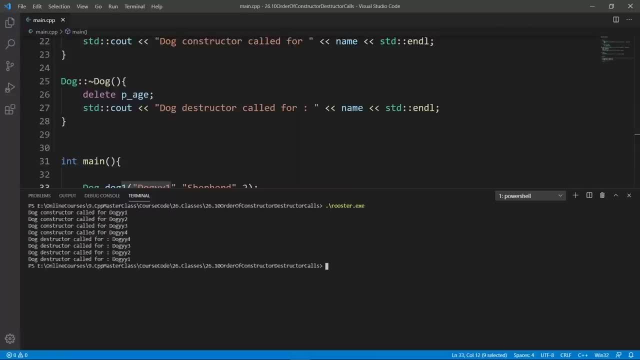 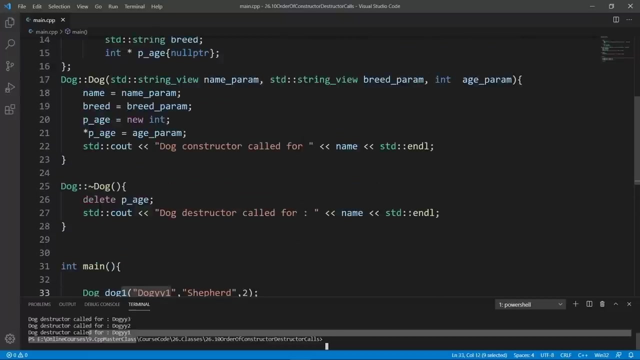 this. let's clear and run rooster. you're going to see that dog constructor called for doggie one all the way to doggie four, and now we have the dog destructor called from doggie four all the way to doggie one, and the compiler is going to enforce this order for calling constructors and 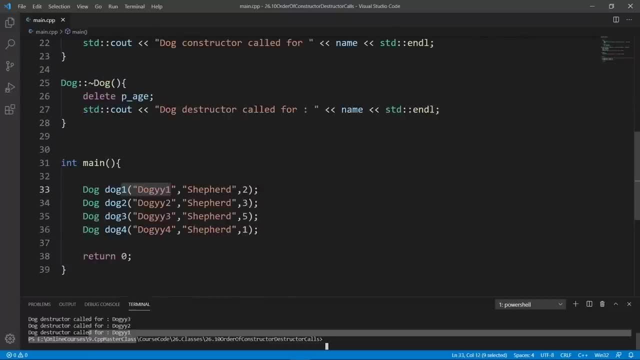 destructors because it makes it easy for it to manage the memory of objects. for example, if dog one has been around for a long time and it has because it's going to be around before dog one, if you delete dog one after dog four here there might be other objects that 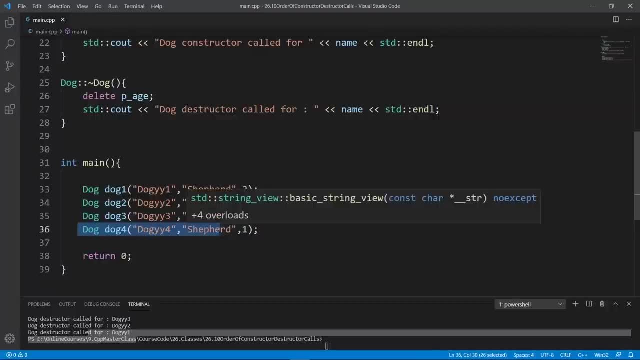 depend on dog one. so that's why the object that was created last is deleted first, because chances for other objects to depend on that last object are really slim and you can delete without any problem. but the object that was created first might have other dependencies and you're going to be deleting dependent object first before you delete that object. i think this. 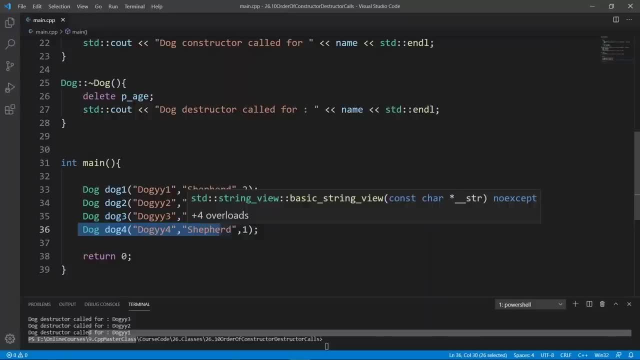 is the logic the compiler follows to really enforce this order here, and you need to be aware of that and make sure that at any time in your c++ application this is working to your advantage. this is really all i had to share in this lecture. i hope you found it interesting. 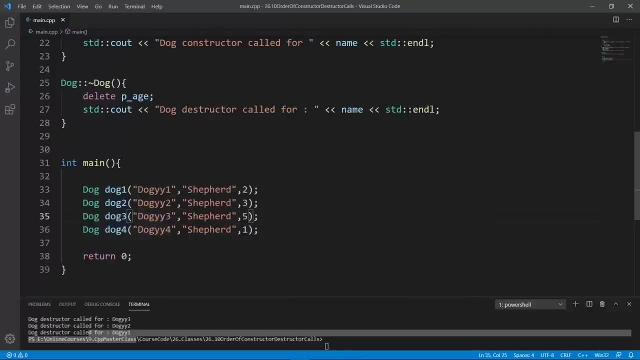 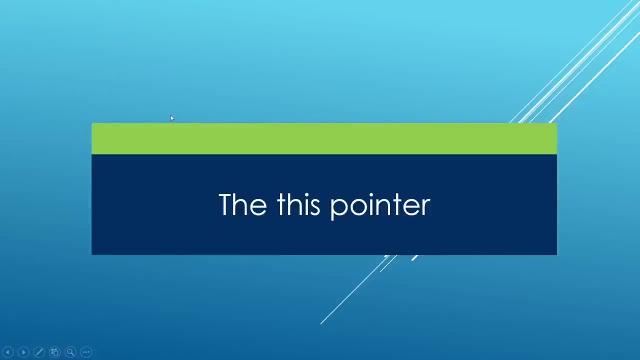 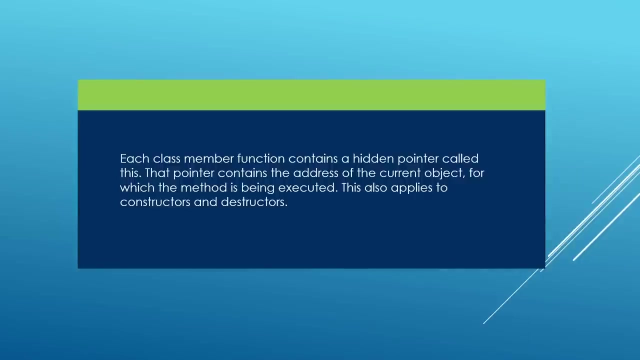 we are going to stop here in this one and the next one we're going to learn about the this pointer. go ahead and finish up here and meet me there. in this lecture, we're going to learn about the this pointer- and this is a special pointer that is maintained by c++ to really 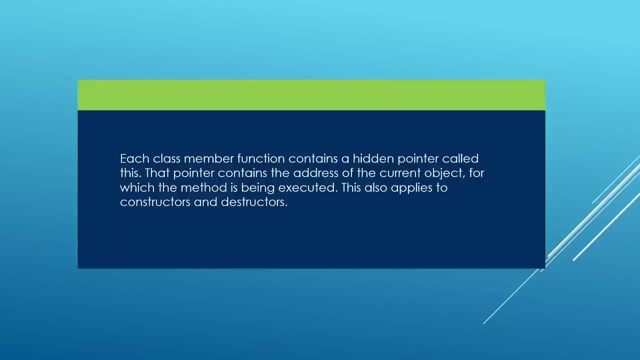 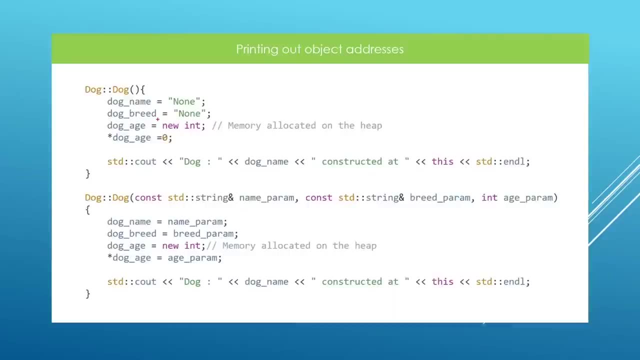 help you manipulate the current object, and it is the current object for which a given method is being executed. here is a simple example with our dog class and we're going to show some usefulness for the this pointer. the first thing we're going to look at is the syntax. for example, here we might need to print the address in memory. 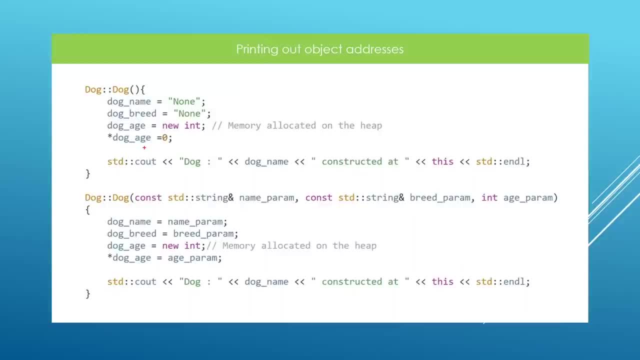 where the object was created and do that from the inside of the function. and to do that we use the, this pointer. for example, we can put out a message and we can do that through a statement, like we have here. we are printing dog, dog name constructed at a given memory address and we use this keyword. 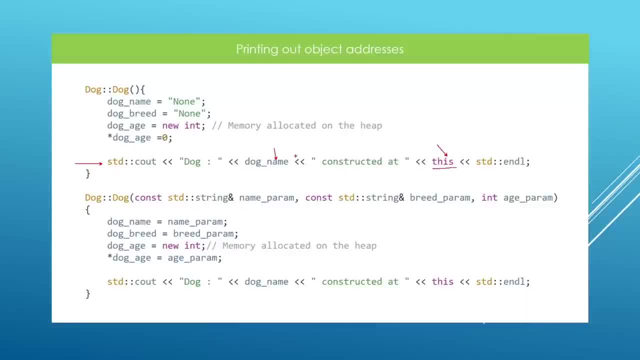 to get the address of the current object for which a specific method or function is being called. in this case it was the constructor of the dot object. here we can also do the same thing for the other constructor. and you see, we are using the this pointer. this is one of the uses you have for 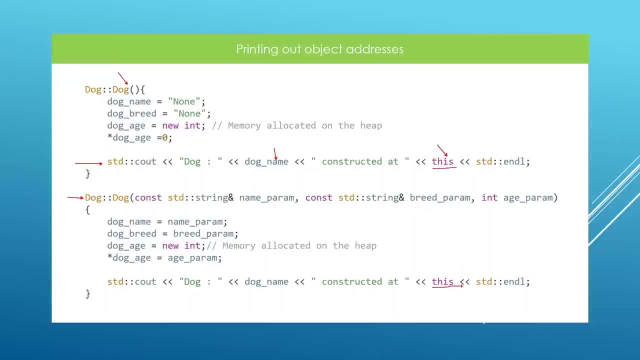 the this pointer again. the this pointer is a special pointer that is maintained by the c++ system and it is going to be pointing to the current object that is being manipulated by the c plus plus runtime and it's going to be manipulated through a special function of the class object. 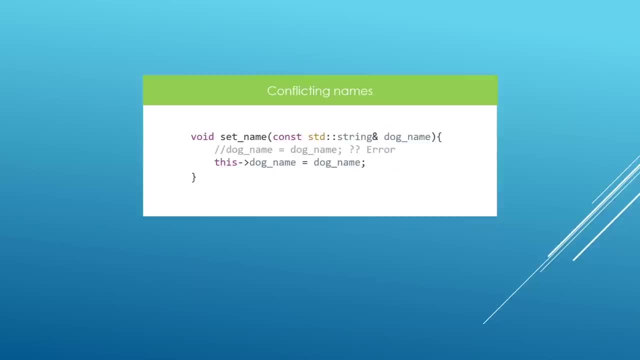 that is being called. this is the meaning here. here is another use case for the this pointer. it may be used to resolve conflicts when you have a parameter and a member variable that are named the same way. for example, here we have a parameter, here we have a class object, and we can use this to. 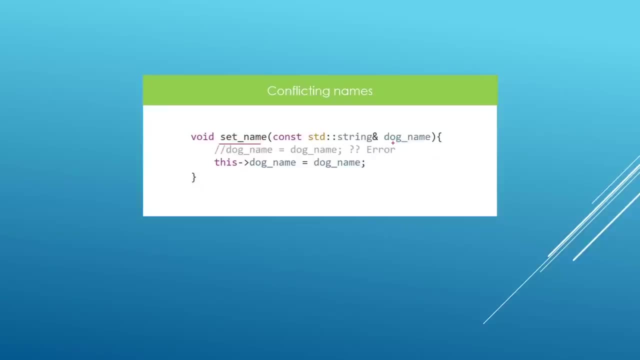 called these class objection to the once system. so by creating a class objection for this, this IP, today the class object is being called here. so in the preparatory provided by a operator which is called are calling the set name function. it has a parameter with a name- dog name- and it has a 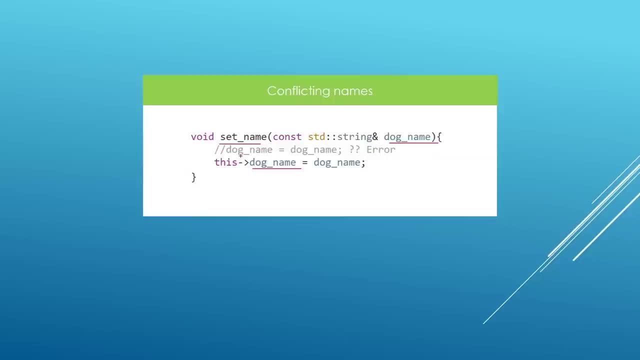 member variable called dog name. so if you do a statement like we have on top here, the compiler is going to be confused. you're going to say dog name equals dog name and it won't really know which duck name you are referring to. we can resolve this conflict by saying this and say: 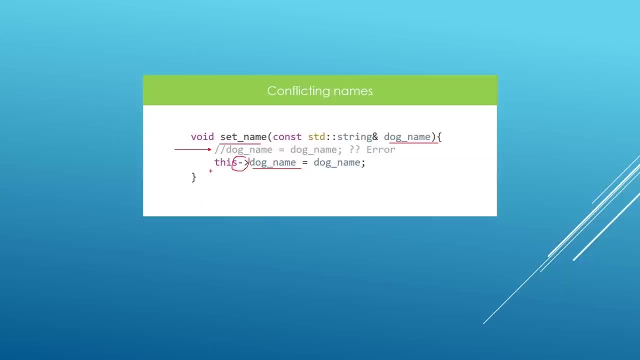 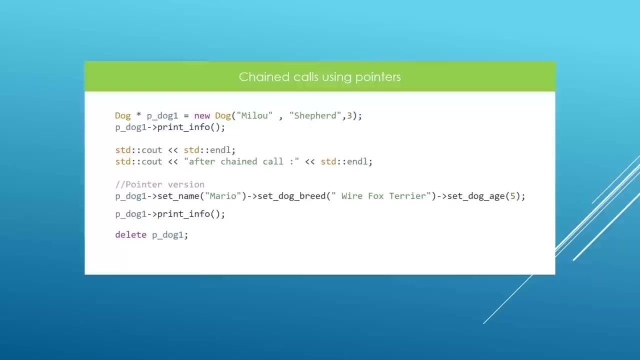 pointer access notation and say dog name, and this thing here is going to be the member variable and we're going to be assigning to the member variable from the parameter. this is the meaning here and we can use the this pointer to resolve such conflicts. another use we have for use pointer: 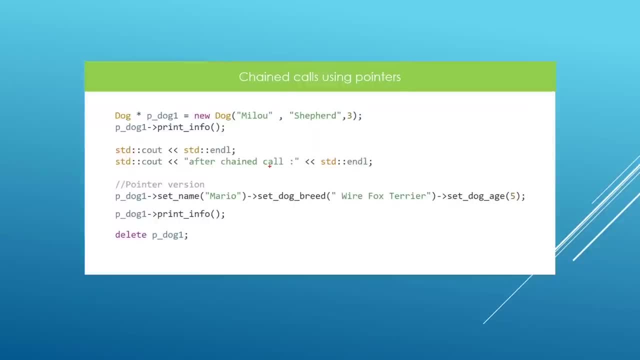 is if we want to set up change calls, for example, using pointers, and we might need to do something like this. so we have a dog pointer set up on top here and we can do something with our new object. for example, we can call a function called printable on our dog object. 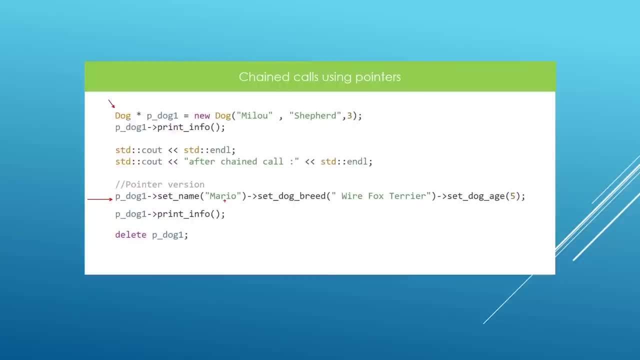 after we've printed the information, we're going to set some information on the dog and, you see, we are setting all of the information through one statement. the way we achieved this. our setters are going to be returning a pointer to the current object and we're going to be 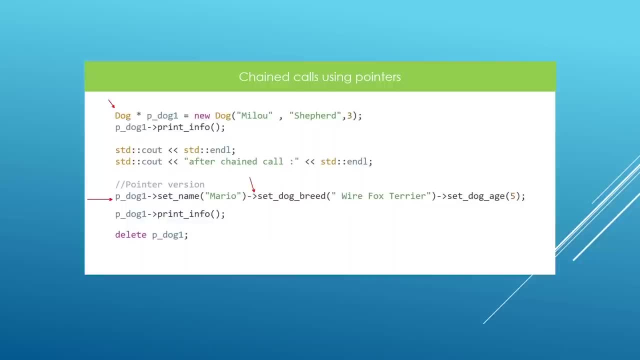 grabbing that return value and calling stuff on it directly because it's a pointer and we are going to be using the pointer access notation. so we're going to call set name. set name is going to return a pointer, we're going to use that pointer to set the breed and set breed is going to return. 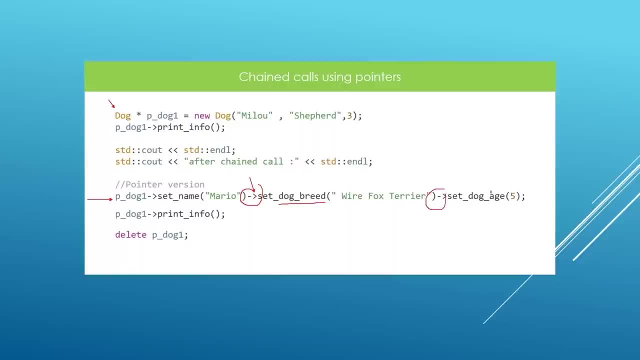 a pointer. we're going to use that pointer to set the age and after this entire line, all the information is going to change about our dog and we can see that here and after we do whatever we want with our dog object, we're going to release it from memory. so this is another thing you can. 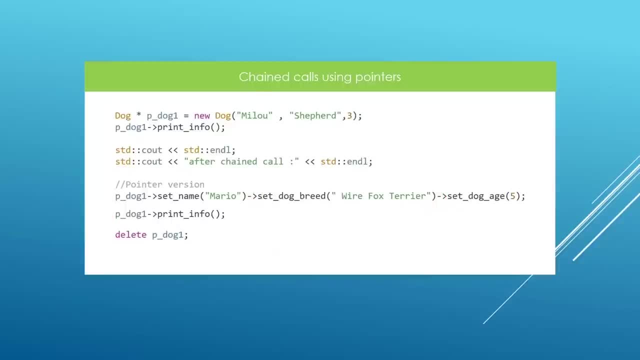 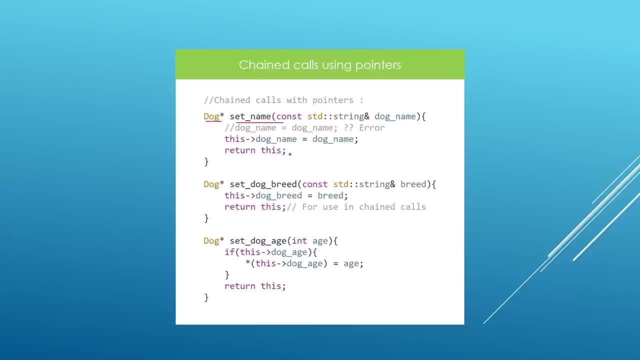 achieve using the this pointer and this is how you can set up these setters. it is nothing complicated. we have set name, it's going to return a dog pointer and we're going to return this. okay, and this is going to be a pointer, or the memory address of the current object of the dog class. 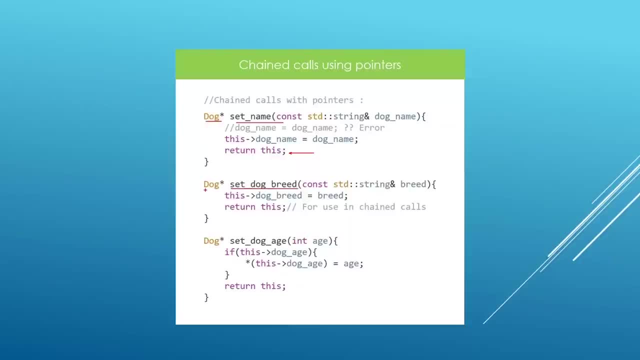 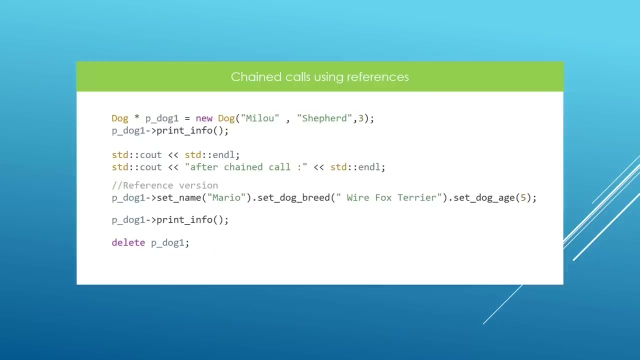 we have the same setup for set dog breed: we return the dog pointer and we return this. the same setup for set dog age: we return a dog pointer and we return you this. we can do the same thing using references, but our setup is going to be somewhat a little. 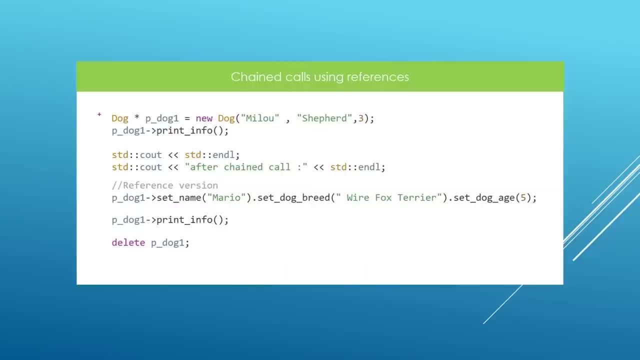 bit different. we have our dog object here and we're going to do our chain decal here. so we're going to say set name through the pointer because we have a dog pointer here, but after that we're going to return a reference from the functions here. so set name is going to. 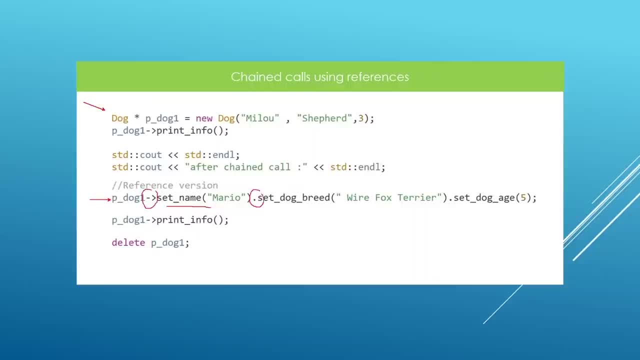 return a reference. we're going to go through that reference to set the breed. set dog breed is going to return a reference and we are going to go through that reference to set the dog age and if we print the information now, we're going to see that we have new information. 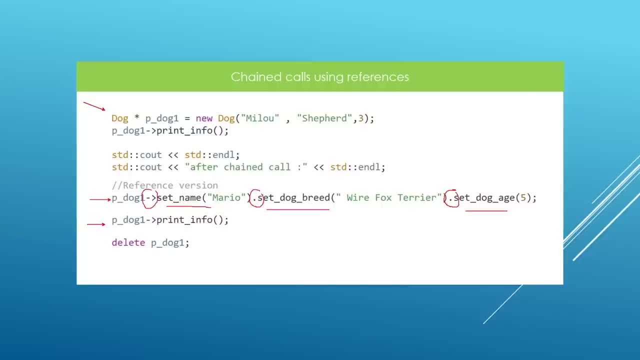 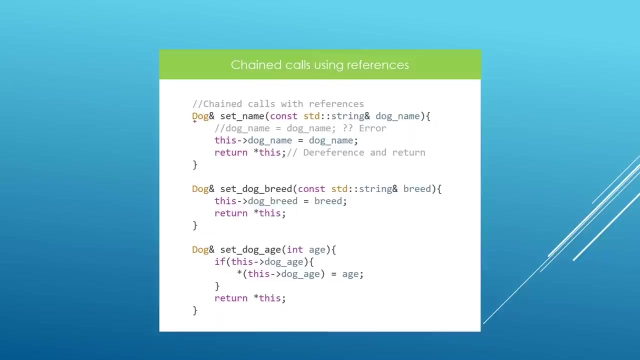 in our dog object and after we are done with our dog object, we have to remember to release it from memory because it was allocated dynamically from the heap. here is how you can set this up. it really is nothing complicated. we just have our setters and we are going to go through that reference to 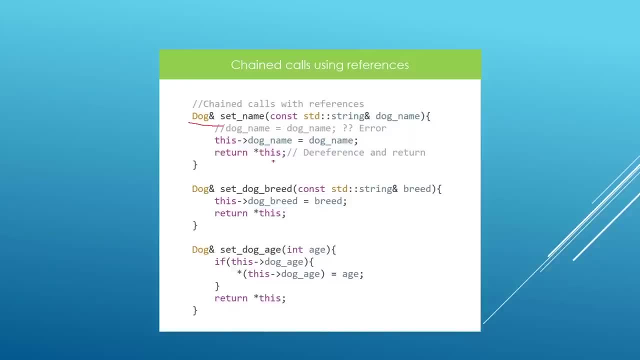 set dog price use this whole bunch of referenceồ. we are using our set dog undefined prefix calling dog and we are going to return a reference. but before we return through the this pointer, we will need to dereference the disk pointer and get to the actual thing that is being pointed to. that's 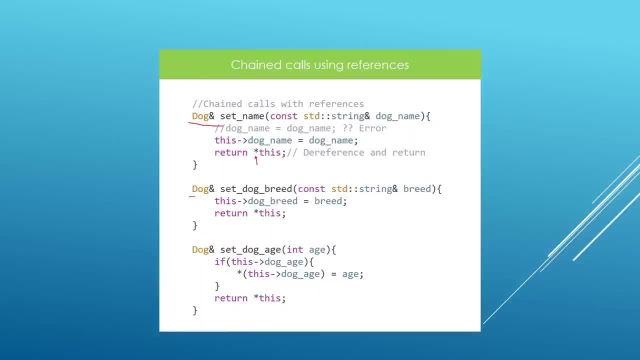 why we have this star operator here. and for the others headers, we're going to do the same thing. we're going to return a reference, we're going to return a dereferenced version of this. we're going to return a dog reference for cit, dog h, and we're going to return a dereferenced this pointer. 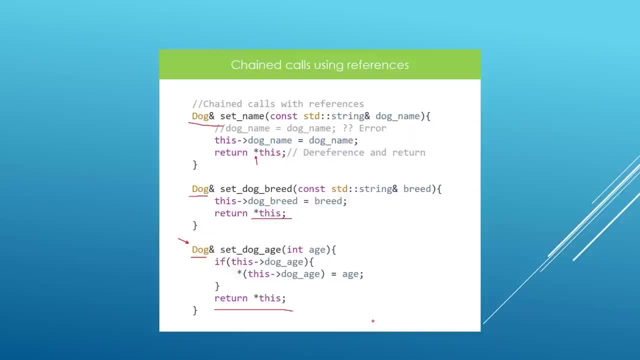 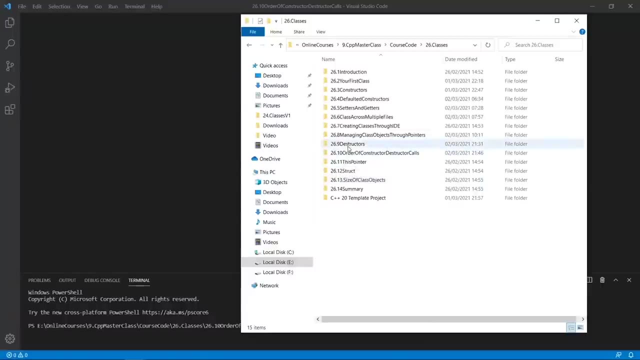 we are returning here, so this is what the this pointer is about. now we're going to head over to visual studio code and play with this a little more. okay, here we are in our working folder. the current project is the this pointer. we're going to grab our template files and we're going to put 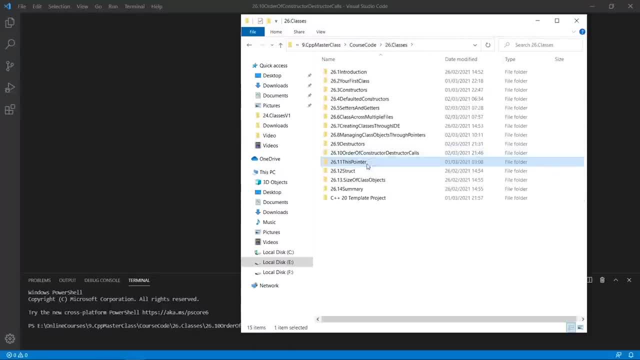 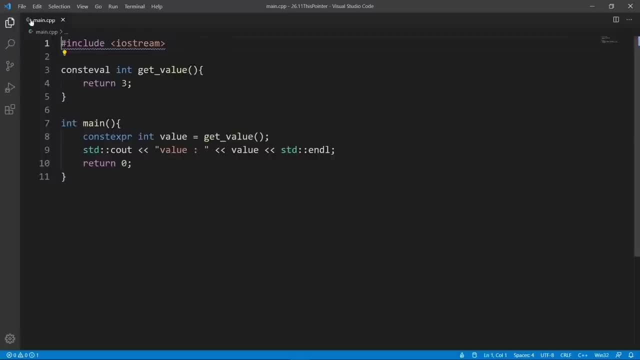 them in place and then we're going to open this in visual studio code by dragging and dropping here. this is going to open our folder, we're going to open the main cpp file and we're going to close the left sidebar here so that we have some more space to work with. i am going to put in a version. 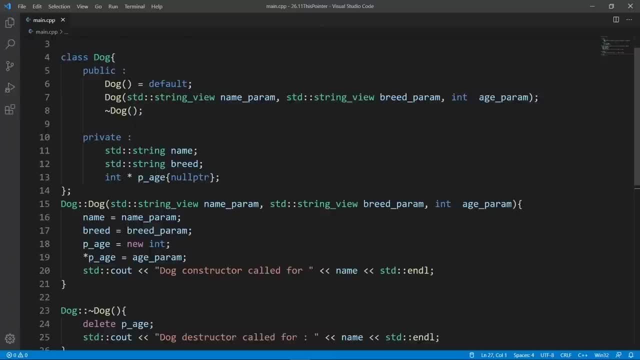 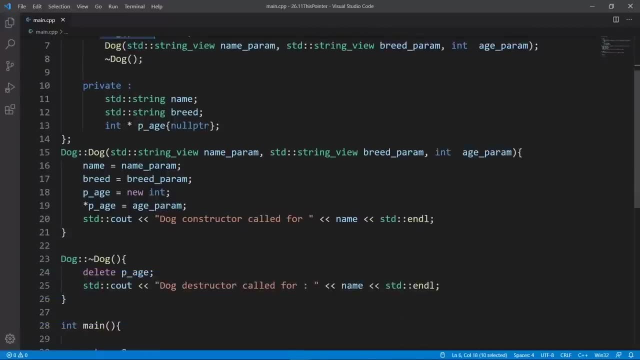 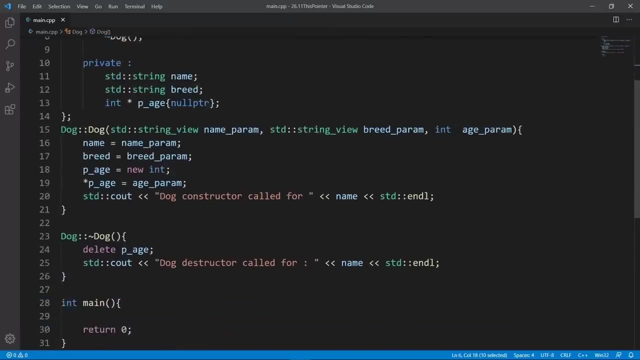 of our dog class. it is pretty limited right now. it just has a destructor and a constructor and a constructor, and we have our member variables and we're going to tune this a little bit so that we can work with us. however we want, the first thing we want to do is to print the addresses. 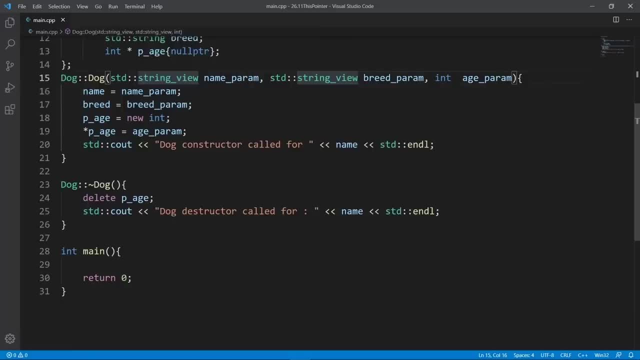 of dog objects that we construct and destruct here and we're going to do that in our constructor. so let's go to our sddc out statement here and we're going to say at to mean the memory address where the object was constructed and we're 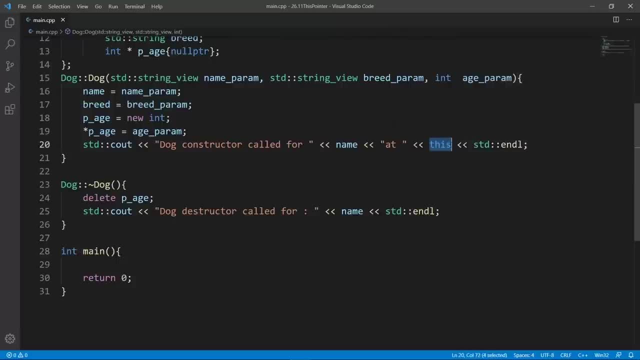 going to say this. so when we do this, this is going to be the address in memory of the current object that is being constructed by our constructor here, and we're going to say the same thing in our destructor. we're going to say at, and we're going to say the memory address where the current object is being destroyed from. 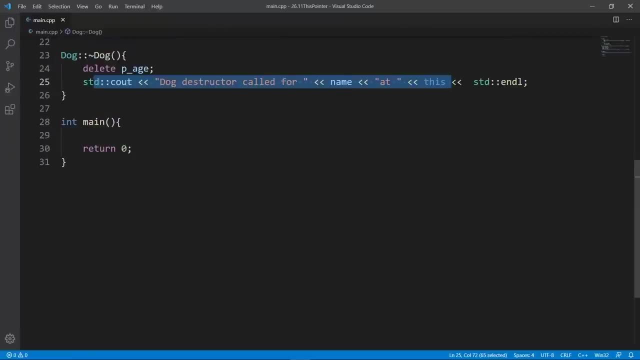 so, after we do this, if we go in the main function and, for example, set up a dog object, we're going to say dog, we're going to say dog one, and we're going to give it the information. we're going to give it the name, which is going to be fluffy, we're going to give it the breed, which is going to be a. 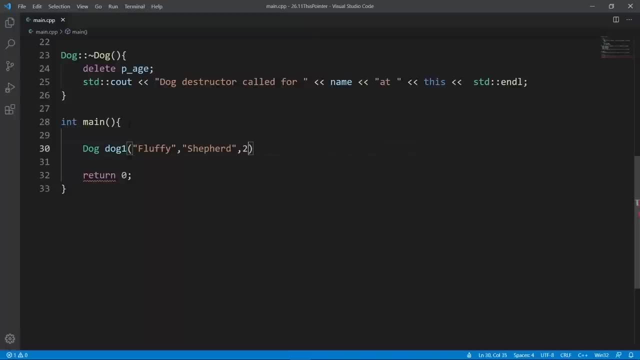 shepherd and we're going to give it the age of two, like we have been doing all along when we do something like this. this is going to call the dog object and we're going to say dog one, and we're going to say dog one and we're going to give it the name which is going to be the constructor, because 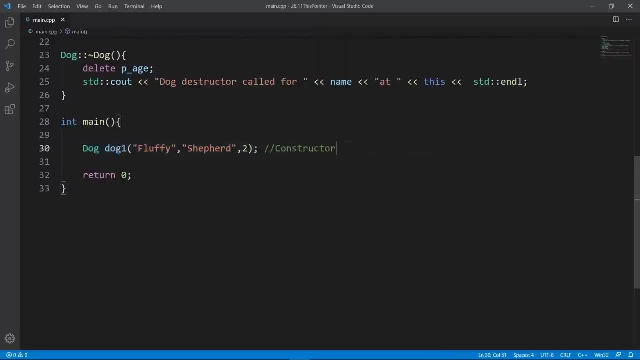 we are trying to set up an object and before the main function ends, we're going to call the destructor and we're going to see things happening here. let's say done, so that we know that the code is actually running. we're going to say: stdc out. done here. okay, we have the setup done, we can. 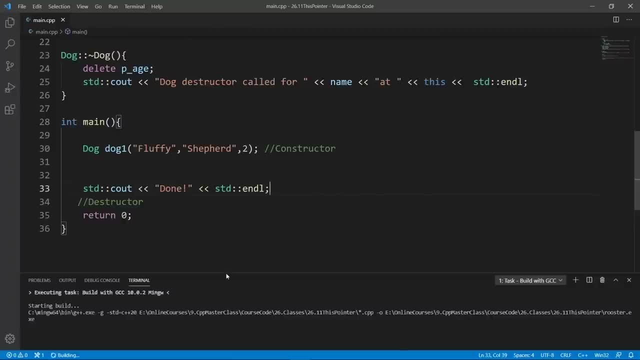 build and run the application. we're going to use gcc to build and the build is good. we can bring up a terminal to try and run the application. and now, if we run rooster, we're going to see that dog constructor called for fluffy at this memory location and the current 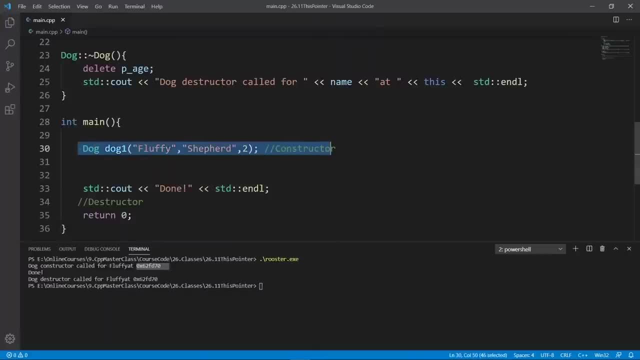 object is this object here which is being constructed and we're going to have access to its memory through the this pointer. hopefully you can see how powerful this is. if we didn't have the this pointer, the only way to get the address to this object would be to grab the address from. 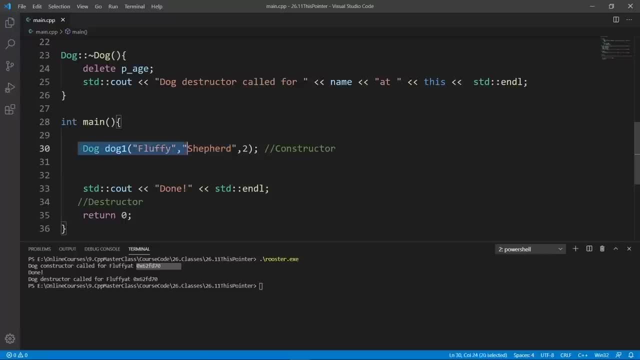 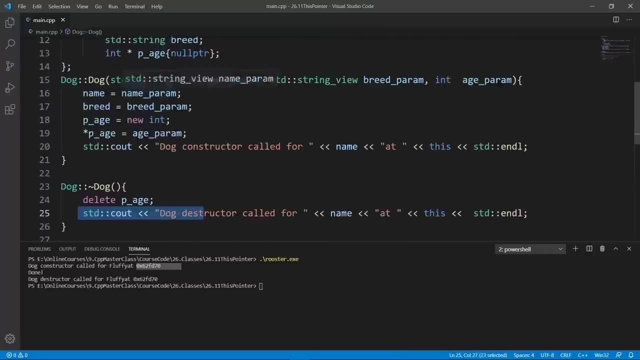 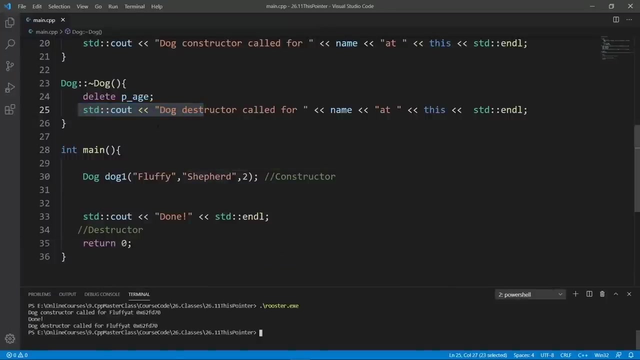 the main function or from wherever we are setting up our object here. but we have access to this address from the inside of the functions for the class and this is really cool. so we can manipulate these addresses if we need to, and we're going to show you another use. 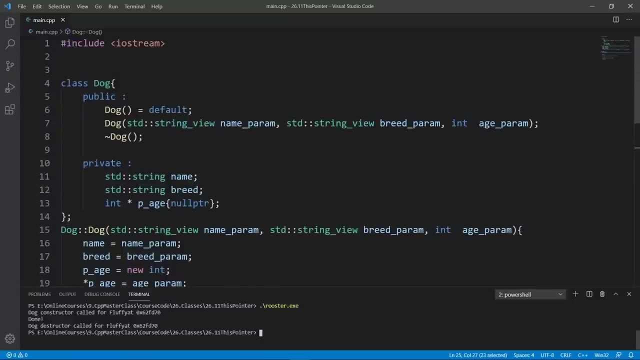 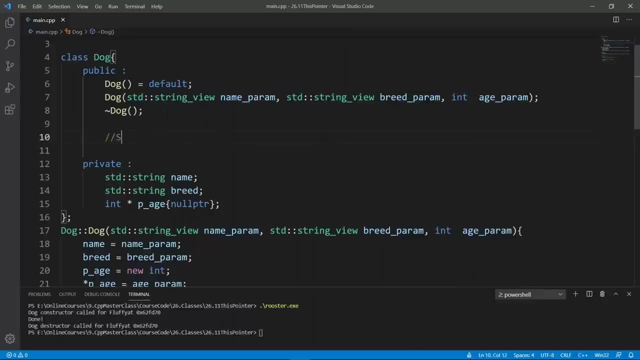 for this. so suppose we need to set up setters for our class here. so we need a setter to set the name, the breed and to set the age here. so let's set up our setters. we're going to say setters and we're going to say void set name. or let's be explicit, set dog name. 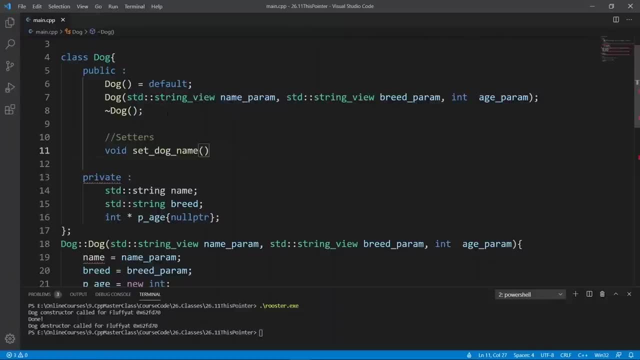 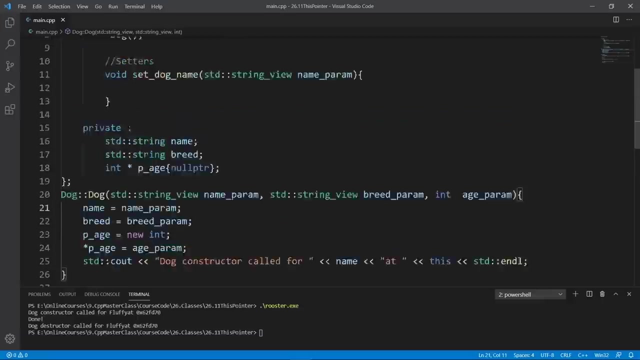 that's going to be better and we're going to pass a string view, we're going to say std string view and we're going to say name param and we're going to put the bodies in our class here. but I would encourage you to be consistent if you are doing this in real code. we are learning here and we are. 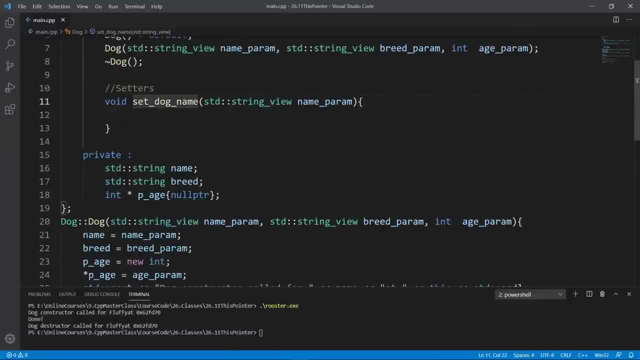 taking some shortcuts so that we can do things simply. but what we want to see now is what happens if we have a parameter named the same as a member of our class. so let's say that we have a member of our variable, so how do you set this name to the member variable called the name? so if you have a 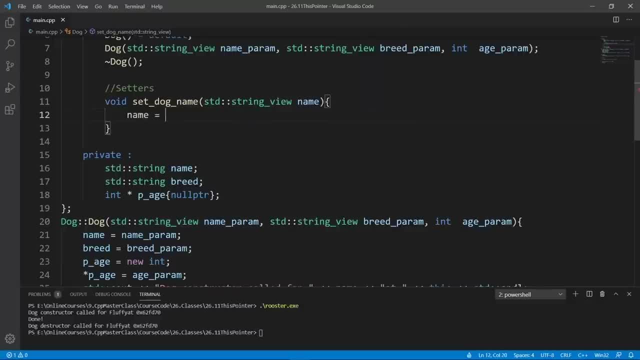 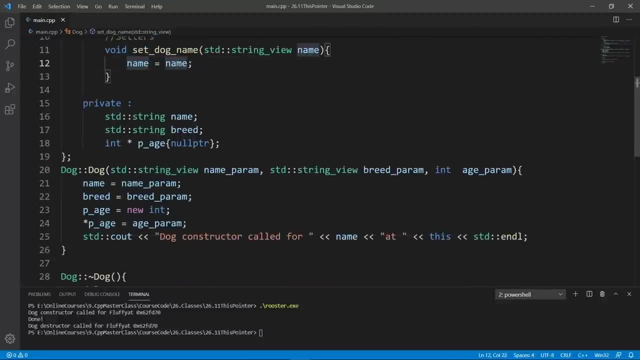 case like this, you're really going to be in trouble because if you say name equals name, let's try this. we should get a compiler error or a squiggly line, because the compiler is not going to know which name are you using here. is it the member variable? is it the parameter? it's not going. 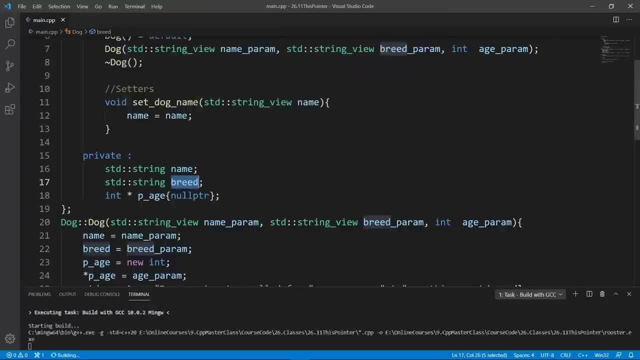 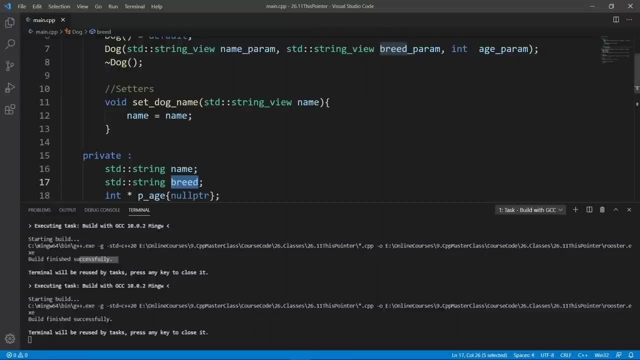 to know and let's try to build and see what we get. we're going to use the gcc and, surprisingly, gcc is taking this and it's probably knowing that we have a member variable named name and it's going to assign the parameter to that member variable. so, behind the scenes, gcc is going to 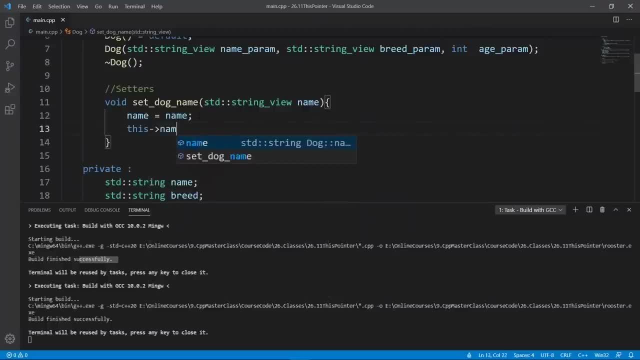 change this to this. it's going to use this: name equals name. this is the syntax we want, which is really not confusing, but what we have on top here is going to be confusing and some compilers are not even going to take this. let's leave this in. 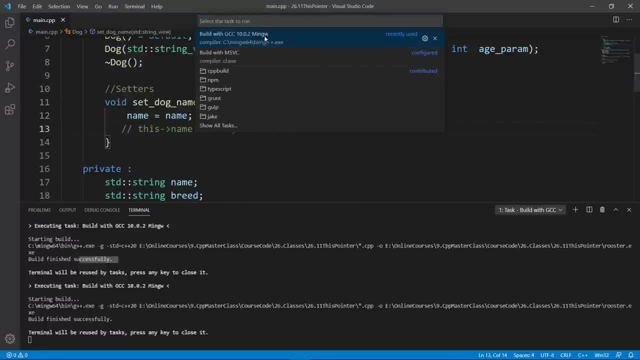 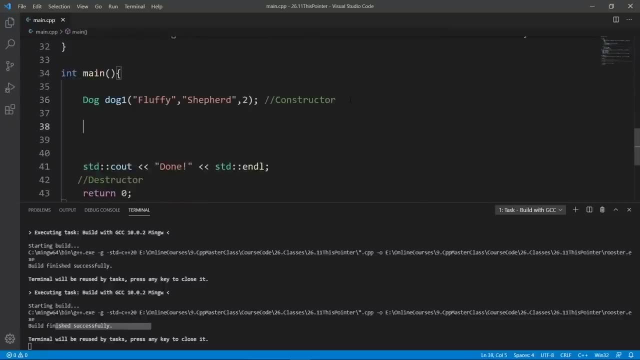 actually build again with us. I want to see that this actually works. so we're going to world successfully. and if we go down in main and try to say dog, one set dog name. let's say pumba, let's see what happens. if we do something like this, we're going to try and build again and the gcc is going. 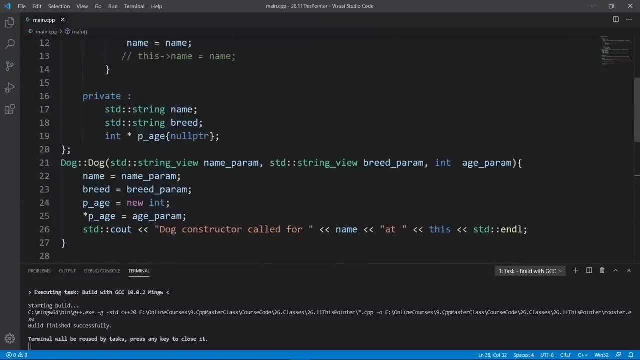 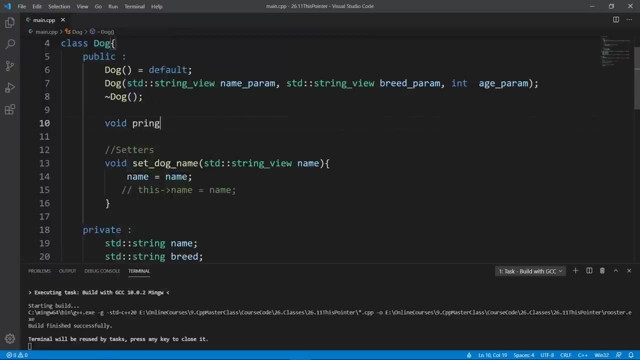 to take this and this is really cool. so let's put in a function which is going to print information about our dog. we can do that down here and it's going to return nothing. it's going to print info and it's going to basically print the name of the breed and the age. so it's going to say: 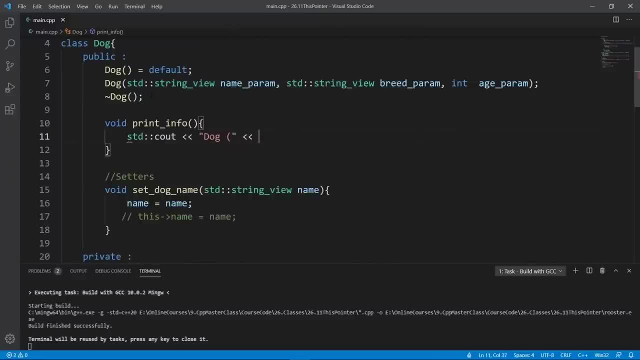 sddc out. we're going to say the address where the dog object leaves. I think that's more meaningful. we're going to say this and then we're going to put a parenthesis and say the name. I think we can put a an angle bracket here and say name and we're going to say the dog name. we can go down and say: 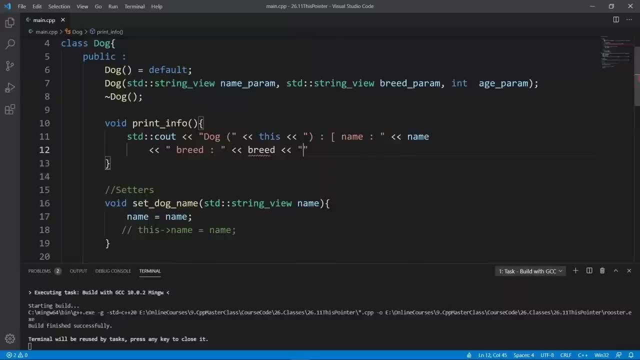 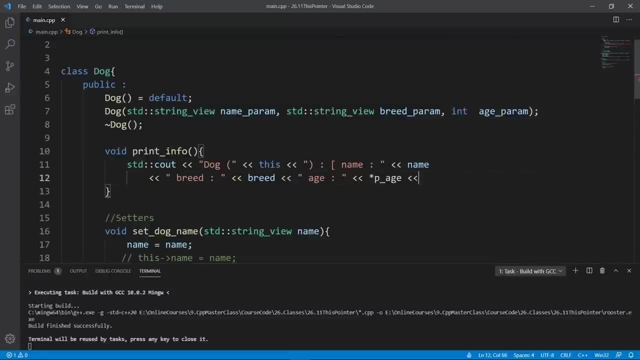 the age or the breed and say the age and we're going to dereference the age member variable because it's a pointer. we're going to say the reference ph here and I think this is going to be at now. we can put a new line character. 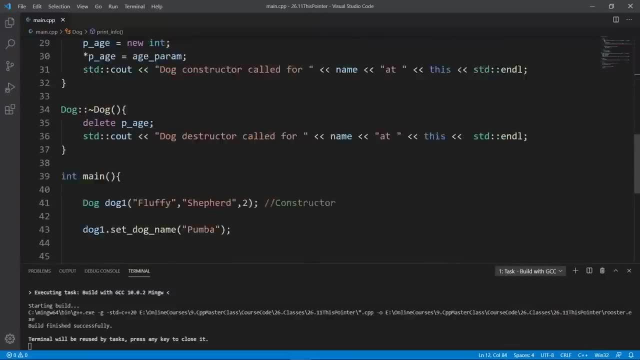 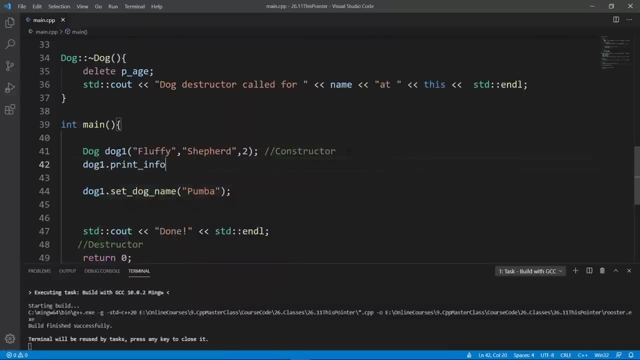 std endl. and if we go down now and say print info, before we set the name we're going to say dog one, print info. we're going to print the information about this dog and after we set the dog name we're going to go down and also say dog one, print info. you can play with this. 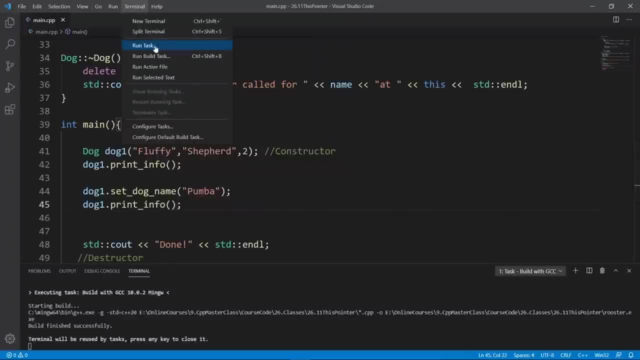 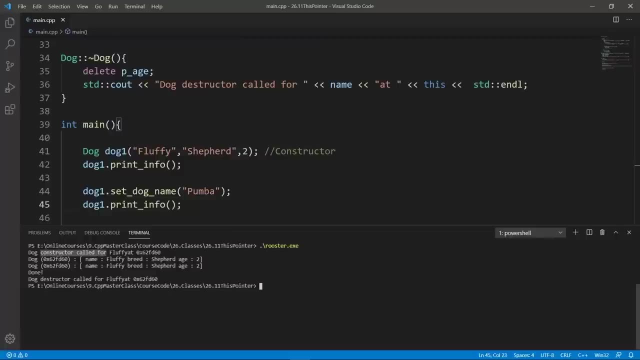 things and I really encourage you to do so. so we're going to build this, we're going to use gcc, so the world is good, we can clear and run rooster. this is going to say the constructor was called for fluffy at a given address. we're going to say the dog. we're going to print the information and. 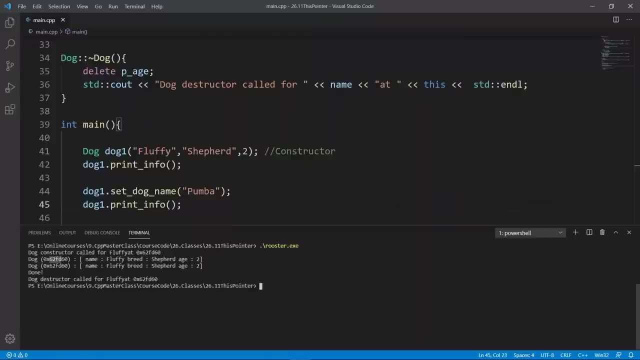 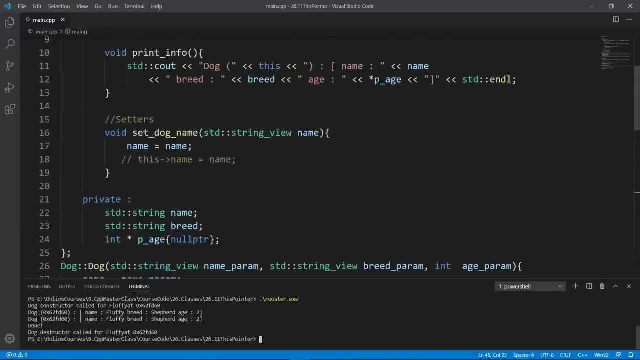 we're going to say it's a dog object at this address. the name is fluffy and we're going to print the dog for the second time. you're going to see that the name is still fluffy and we have a problem here. why is that? why is our object not being modified? let's go up and see our set dog name function here. so we're 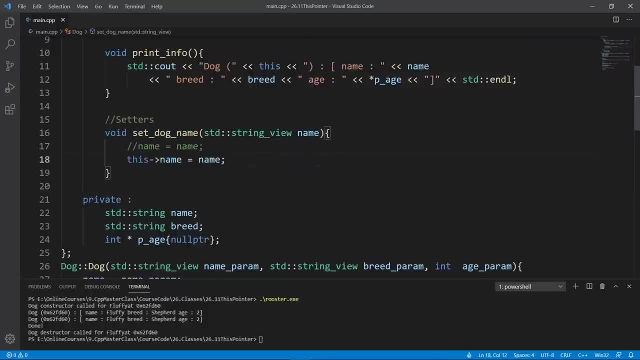 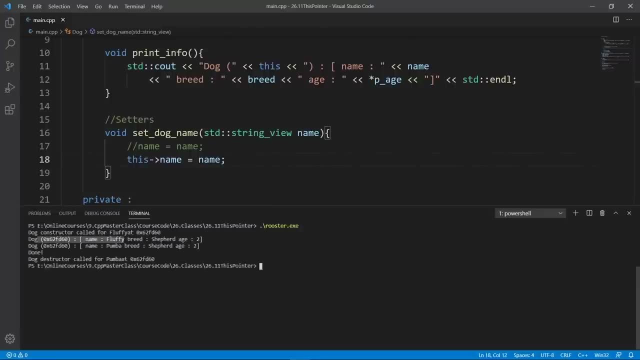 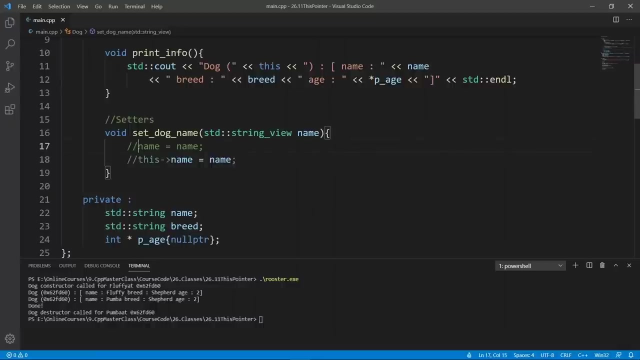 going to remove this and we're going to use the this pointer and we're going to world again and let's clear now and run rooster. and now you see that the changes are actually making sense. so what is happening with the assignment? here the compiler is assigning the value of the variable. 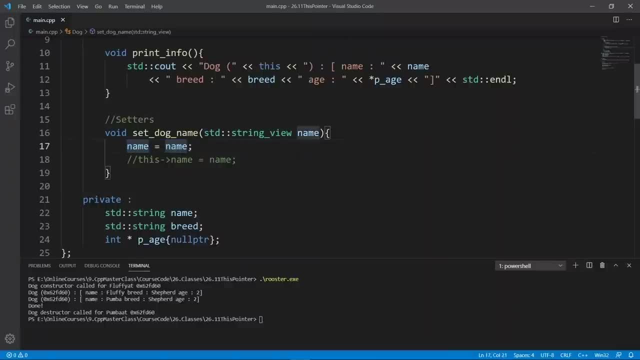 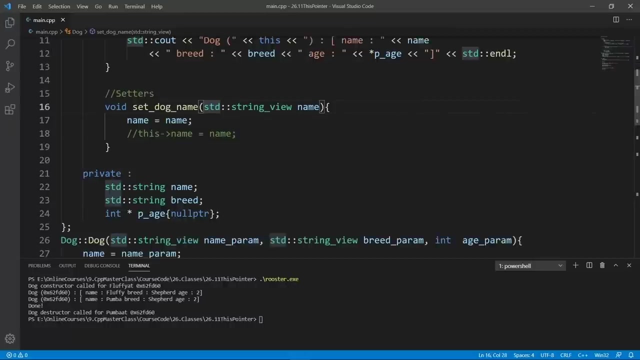 to the variable itself and this is really doing nothing and it is not what you expect. I was fooled a little bit by the compiler because this was compiling, but it's not going to do what you want. when you call set dog name, you probably want to take this name and assign that to the member. variable name of. 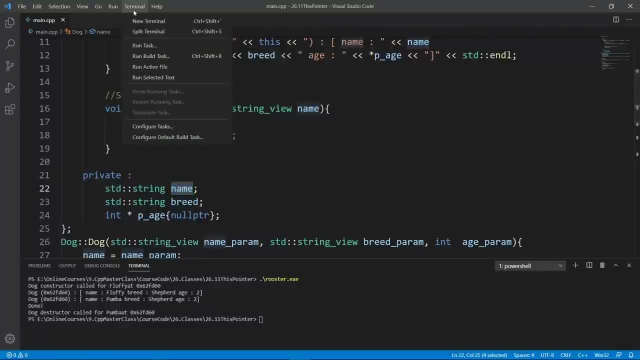 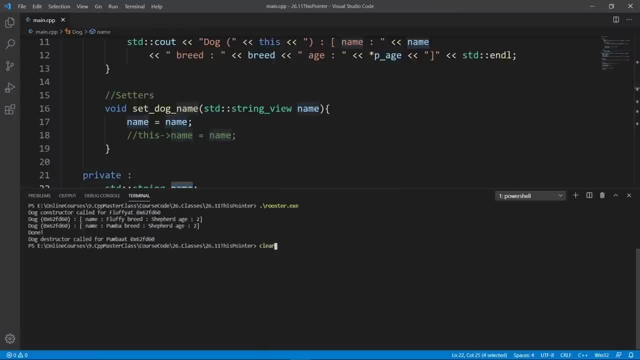 this class, but this is not what it's going to do. let's build again and really show you this. so it is a really good advice to practice and really try things out yourself. we're going to run here. you're going to see that after we set the dog name here to Pumba and we try to print the 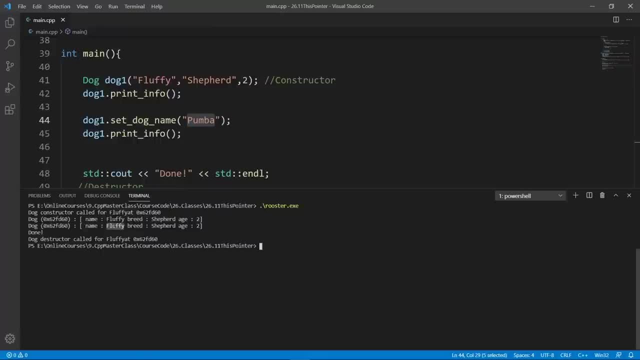 information. the information is not going to be n, the name is not going to be Pumba for the second call here, and what this is really doing is doing nothing here. this does nothing and you really need to know this. if you want to affect your member variable, you will have to go through the this. 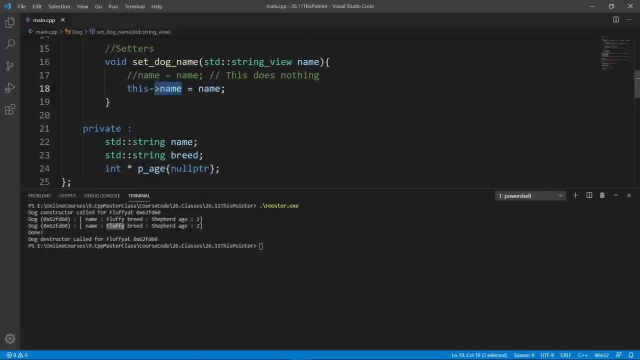 pointer and this is going to tell: take the name member variable of the current object and assign the value in name, the name parameter, to that and that's going to set your name to whatever new name you passed when you call the set dog name function here. so hopefully you really understand this now. if 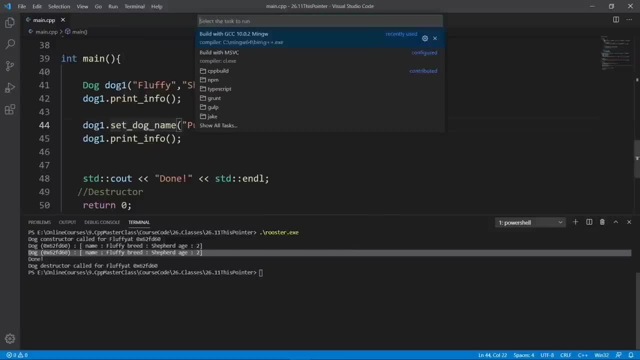 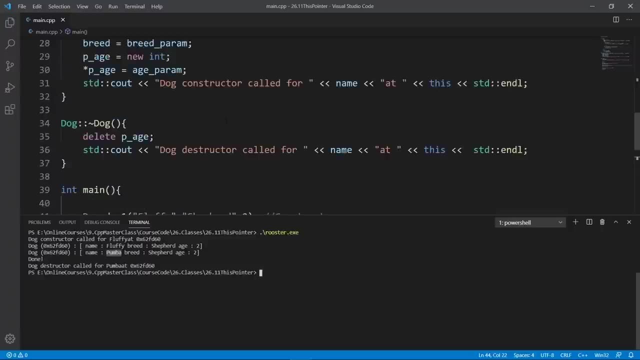 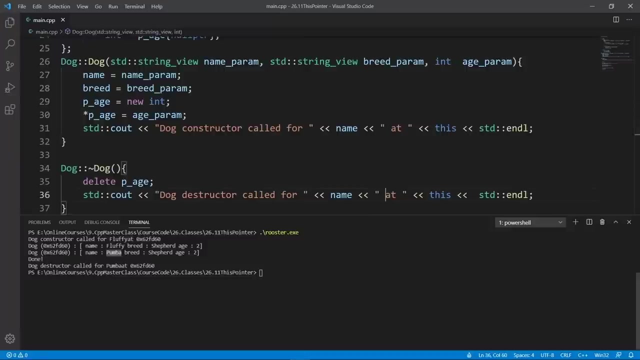 we build, we're going to see that the Pumba name has been applied. let's build again. so we're going to clear and run rooster and we're going to see now that the name is Pumba and there is some annoying thing we have in our constructors. we don't have a space before at here and it is really. 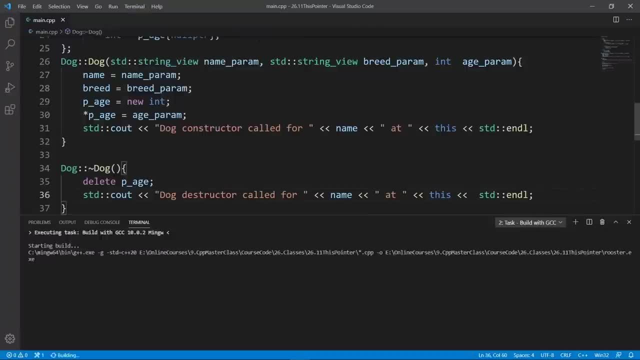 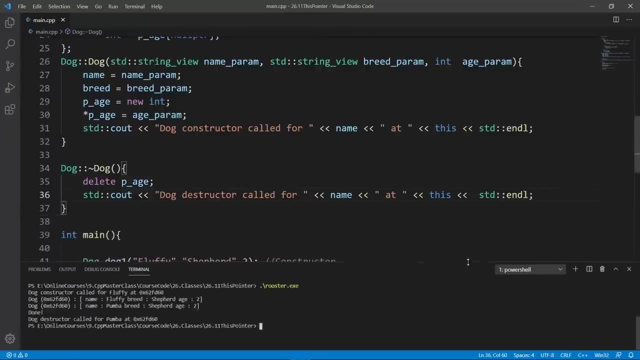 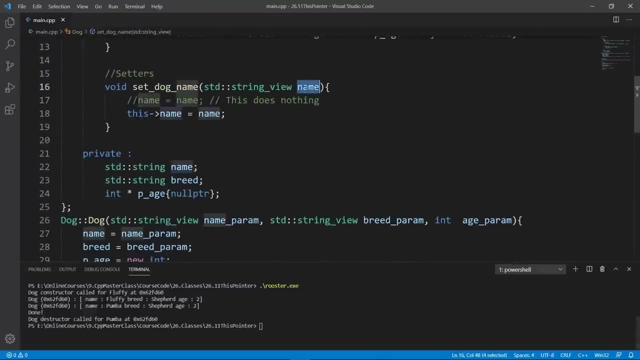 annoying to look at here. so let's build again and fix this. we are going to use gcc. the world is good, we can clear and run rooster and now we have what we want. so this is the second use case you might have for the this pointer, through setters that use the parameter that is named the same as your member. 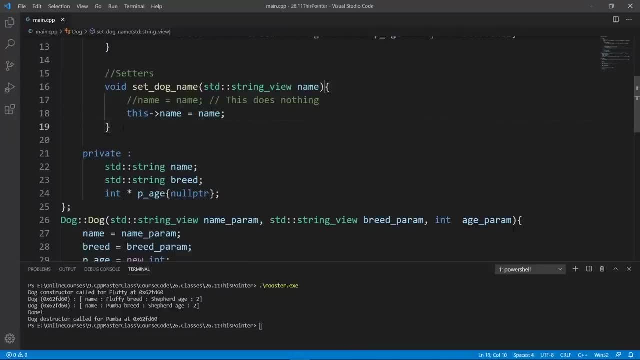 variables. so we're going to set up all the other setters. we're going to set up a setter for the breed. we're going to say std, strength, view, and it's going to be breed. we can do that because now we have tools to really do this properly. we're going to say this breed and 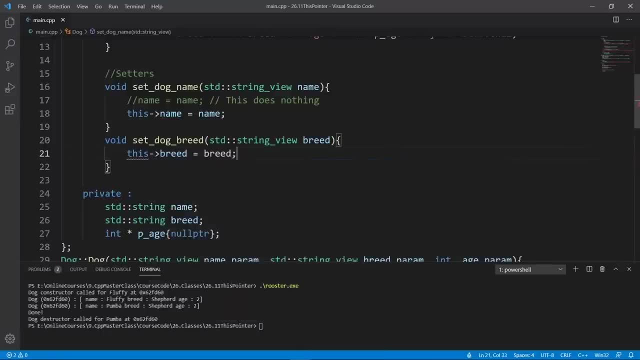 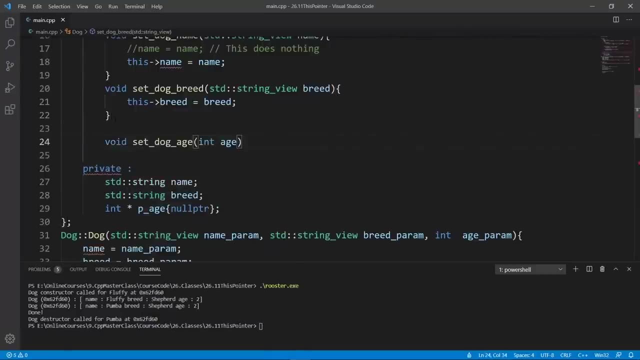 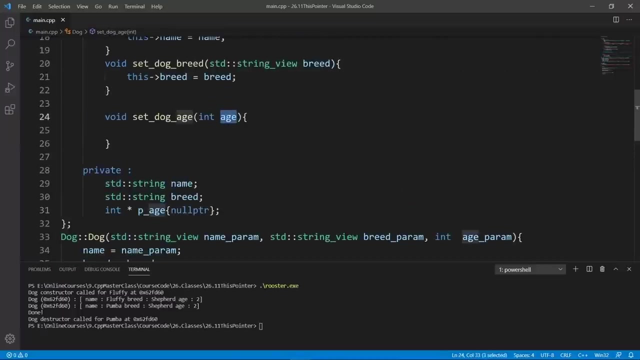 we're going to say equals, read this is going to do and we can set the age. and we're going to say void, set age, dog age. and we're going to pass in a value and we're going to go inside. what is it called? it's called ph. I don't think it makes sense to call the parameter ph, because it's not a pointer. 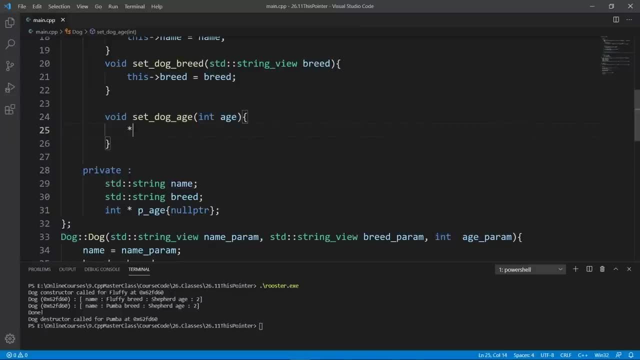 so we're going to go inside and just the reference of a pointer, so we're going to reference that and we're going to say this. so we're going to go inside and say this ph equals age. I think this is going to work and we need to do reference this pointer because what we have as a member variable. 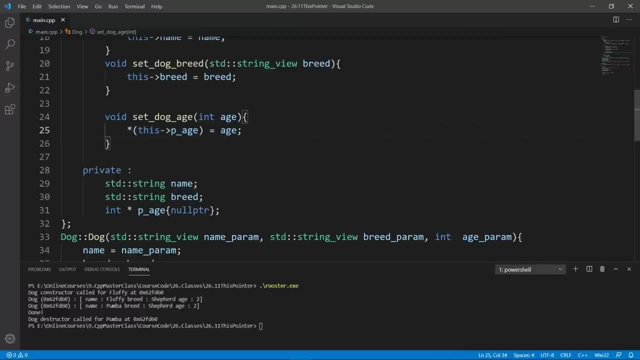 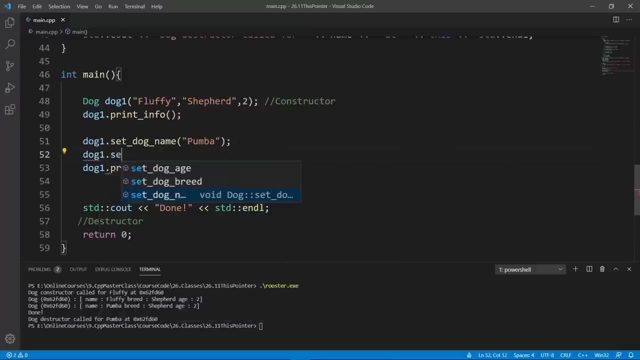 is the pointer. so we need to go through the ugly syntax you see here and this is going to set our age so we can go through this and really change the information. so we're going to change the breed here- set dog breed, let's go down and choose that- and we're going to say wire Fox Terrier and 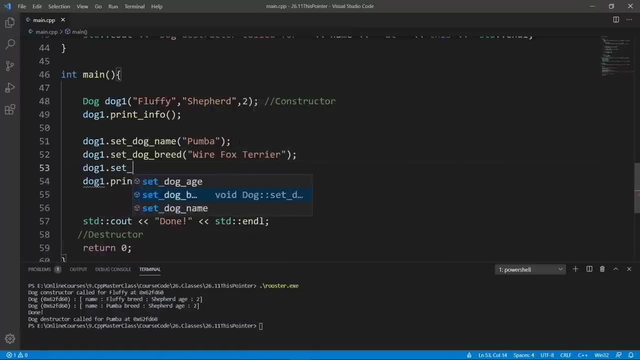 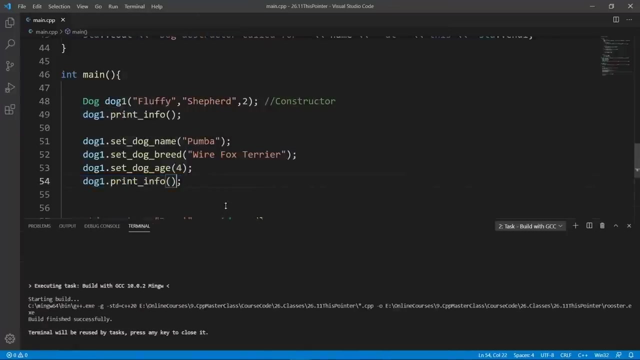 we're going to go down and set the age. we're going to say dog one, set dog age. and we're going to say four, why not? so we change the information of our dog through our setters here and we're going to print new information. let's build again. we're going to use gcc for that. the world is good. 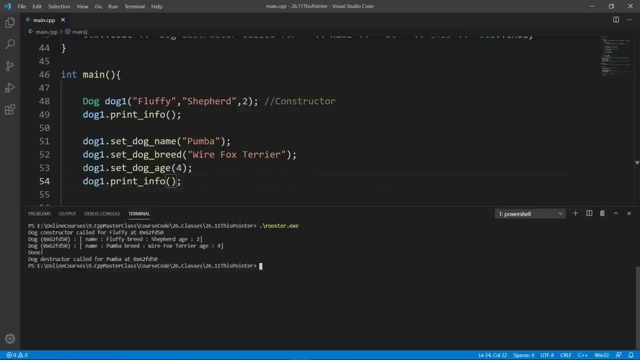 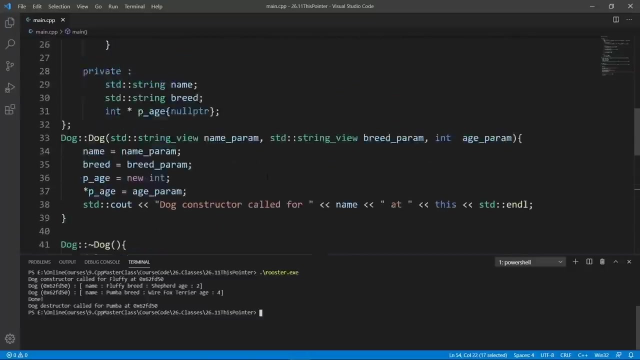 we can clear and run rooster. this is going to give us new information for the second print here. so name is going to be Pumba, breed is going to be wire Fox Terrier and the age is going to be four. and that's the information for our dog object here. okay, now we have this and we want to see how we 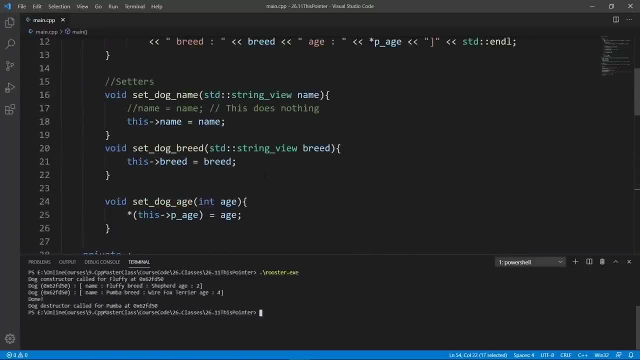 can set up change calls using the this pointer and in this case we will be using pointers. let's change our setters to return dog pointers. we can do that and we're going to go down to say to dog breed: we're going to return a dog pointer and we're going to go to set dog age and we're going. 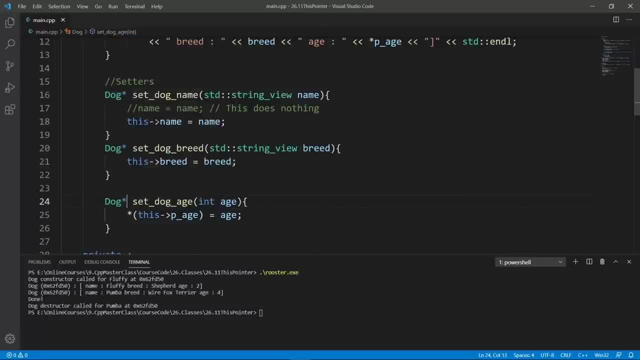 to return a dog pointer. now, after we do this, we will need to return these pointers and we're going to go inside and say: return this. remember, this contains the memory of the current object. so we can return this and fit that to a returned pointer, so we can go down in all the other functions and 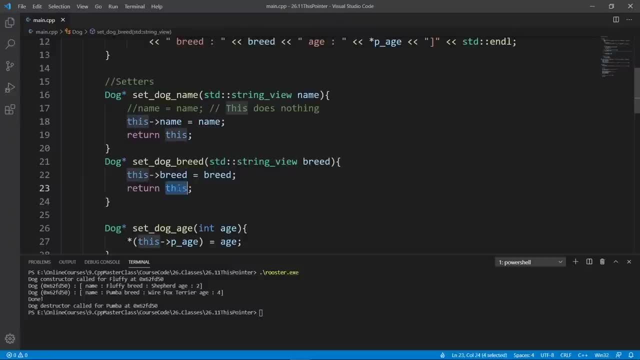 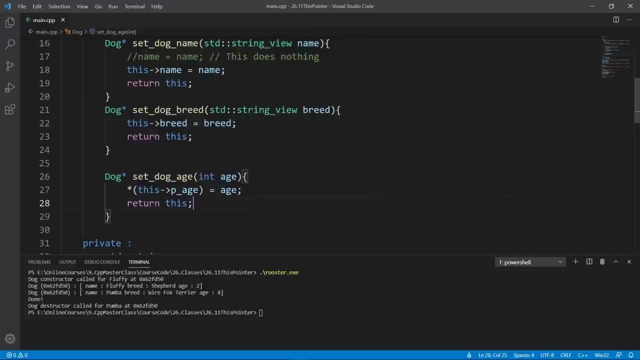 really say this. we're going to say return this. we return the memory address of the current object through the setters that we are doing here. we're going to return this and after we do this, we can change the setting we are doing here. to be one statement, 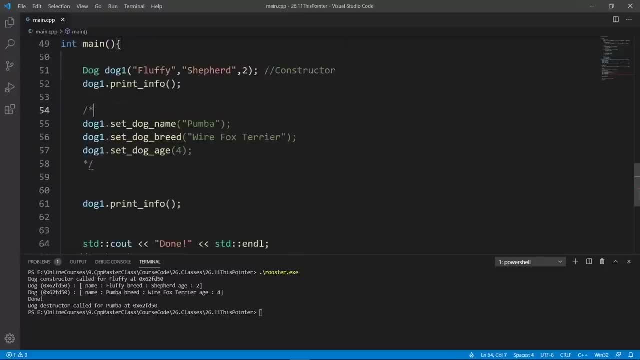 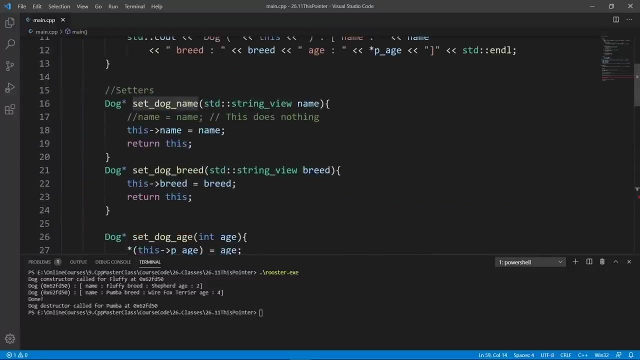 and we can comment this out. I think we can do that- and what we're going to say is dog one and we're going to say set dog name and we're going to pass in Pumba. but this is going to return a pointer now. set dog name is returning a pointer to the current object and you can see that here. 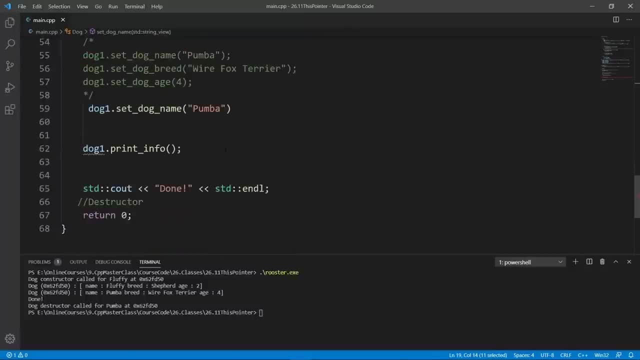 this is what we are returning, so we can go through this pointer and call some other functions. for example, we can say set dog breed directly and a Visual Studio code is going to figure out that what we are returning is a pointer and it's going to change our access notation here to 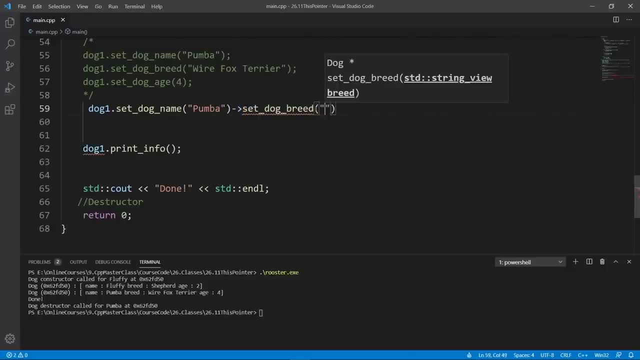 a pointer access notation and we're going to use this in one single statement. so we're going to put in our breed and we're going to call the function to set the age. okay, you see that it uses pointer access notation and this is really cool. so we're going to put in our four and you're going to see. 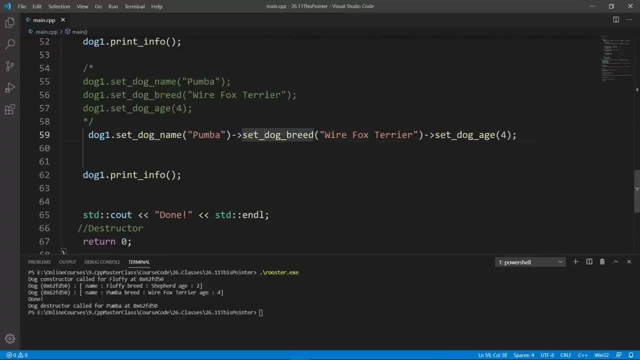 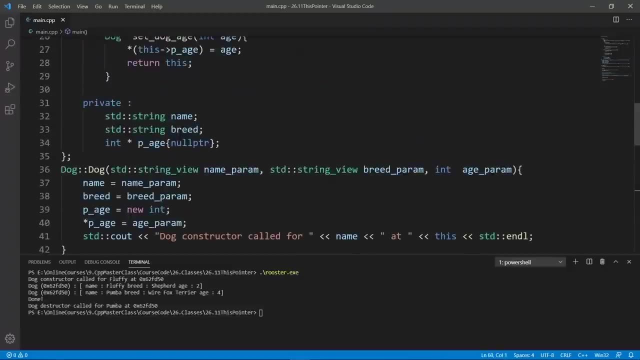 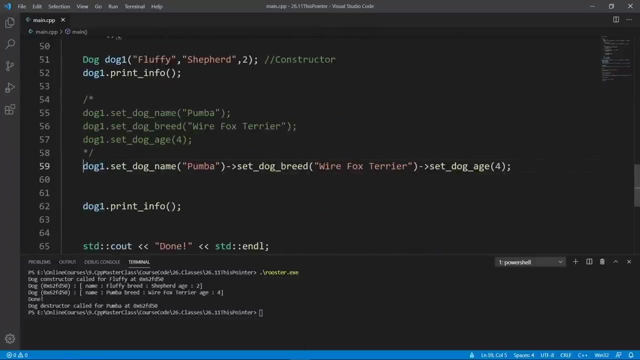 that this actually works and this is really cool. if you don't want to do plans in three steps, you can give your users the option to do things in one step using returned pointers like this, and this is really cool. I use this all the time for my classes that I design in my applications. so if we're both, we're going to see. 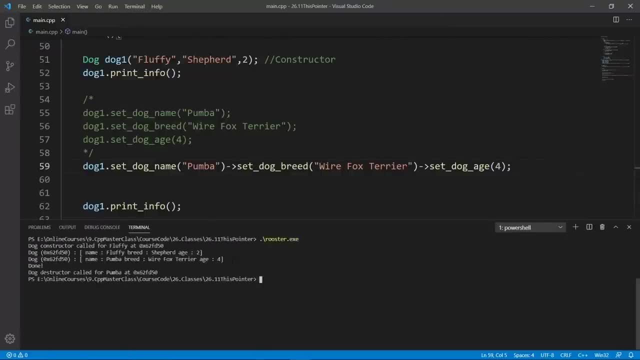 that the world is good and we're going to clear and run rooster. we're going to see that the information is and name is Pumba, breed is water Fox Terrier and the age is four, and we were able to do all these changes in one go, so we can even change this to use. 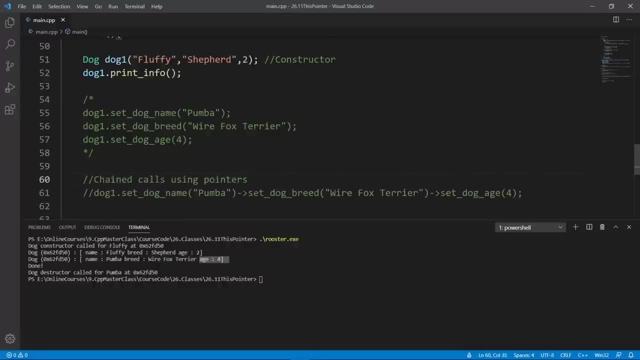 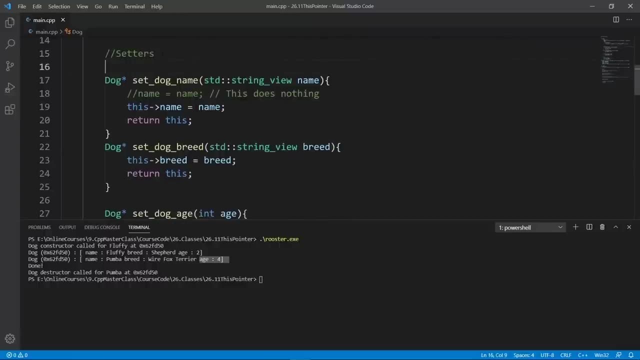 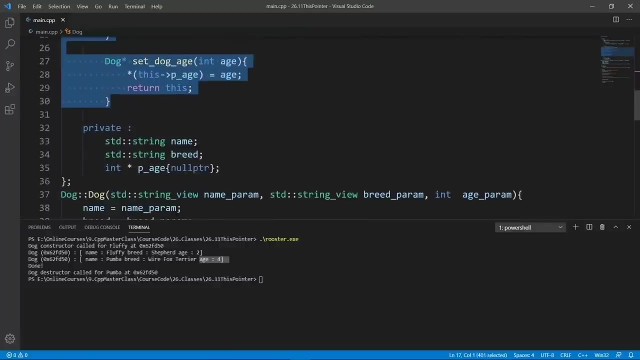 references. here we are using pointers. so let's say that we are using pointers, but we can also use references. let's go on top here and say that this is using pointers and we're going to comment this out, but before we do, we're going to copy all this because we're going to need that and we're 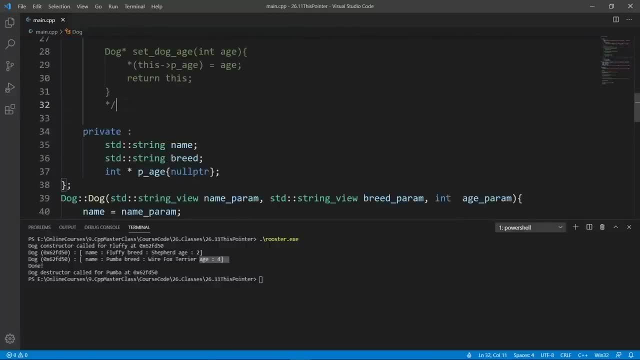 going to comment all this out and we're going to go down and say: change calls using references. and we're going to go down and put in our code and we're going to change our setters to return this instead of pointers. we can do that. so we're going to change the star here to an ampersand. 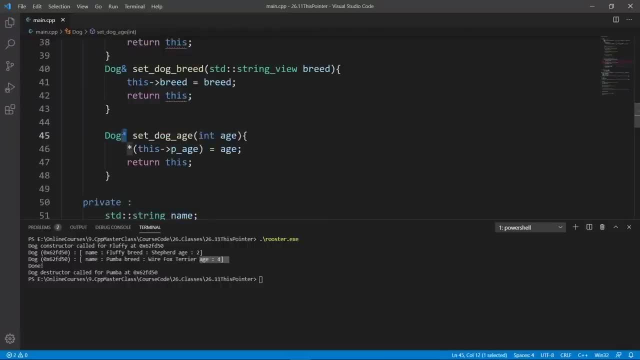 symbol here and this is going to do the magic. so we have a dog reference returned from all these functions. so, because we are no longer returning a pointer- returning this directly is going to give us a compiler error- we need to reference this pointer and get to what, what is pointed to now. 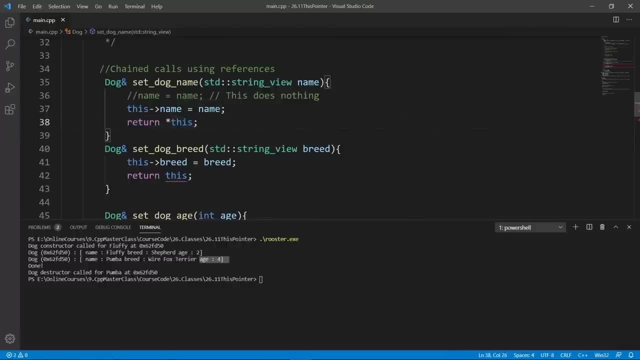 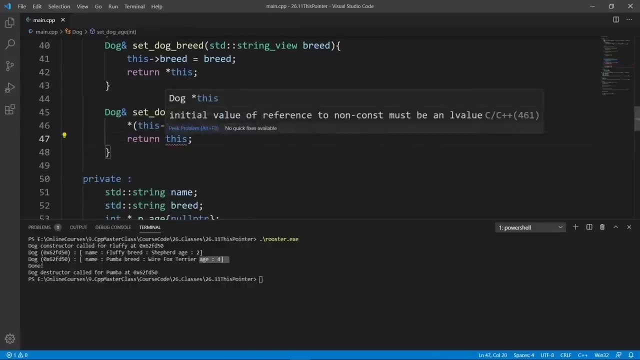 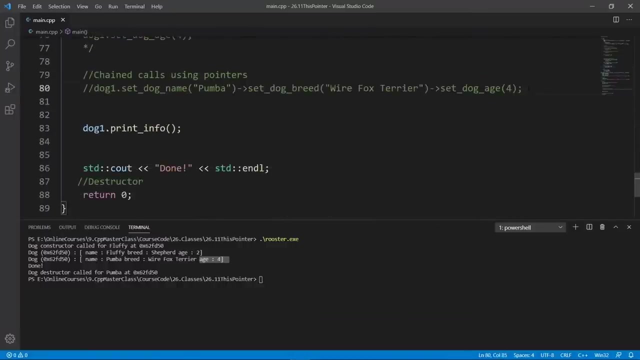 the compiler will know that we are returning a reference to the current object and this is the process. let's go down and the reference or the returned pointers and if we go down, we're going to see that this is good already and we can go down and set up our chained call using references. 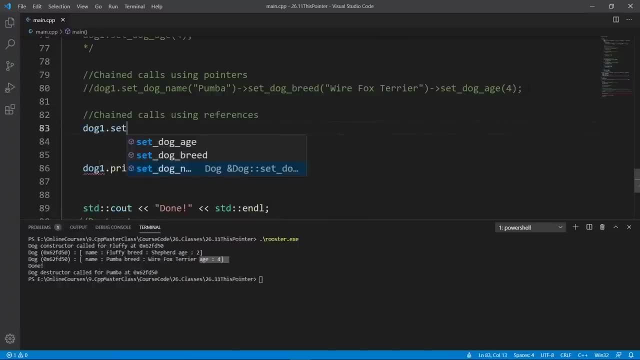 and we're going to go down and say dog one, we're going to set dog name and we're going to pass in Pumba, what we have been doing all along. now we're going to use the dot access notation, because what we are returning is a reference and you're going to see that Visual Studio code is going to bit. 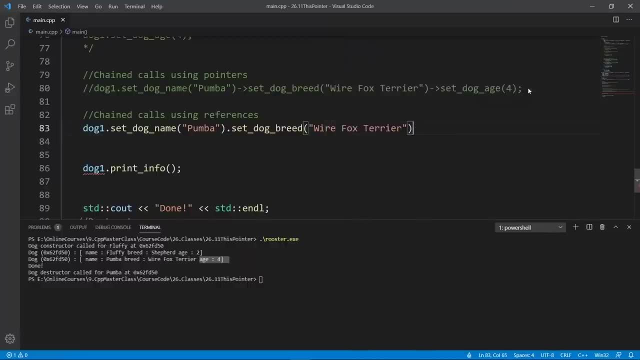 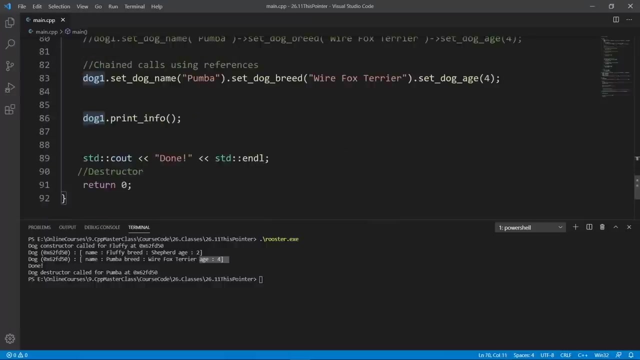 up the breed is going to be Firefox and we're going to say set dog age and we're going to pass in our four and you're going to see that this is valid C++ syntax and if we print the information, we're going to have new information applied to our dog object. here we can world and see that. 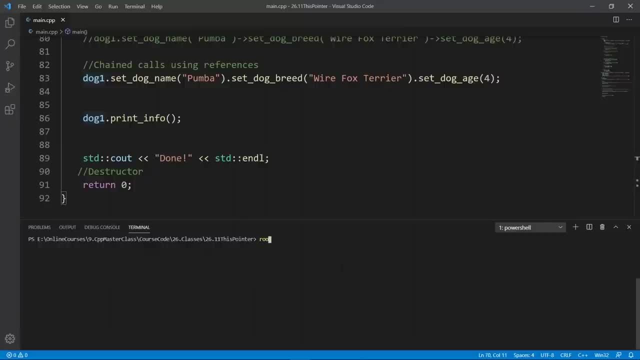 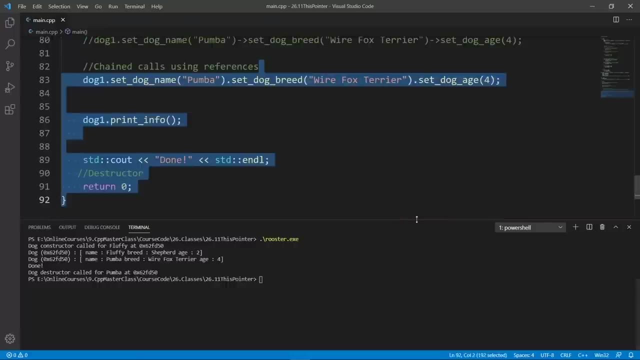 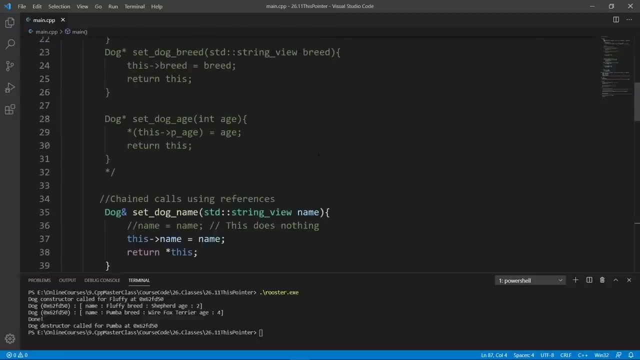 this is actually working. you see, the world is good. we can clear and run rooster and we're going to see that this is quatro, that this is being played right now, and how many do we have to remove from our query, for doing this is automatically gonna dismiss. so we're going to tasting and we have 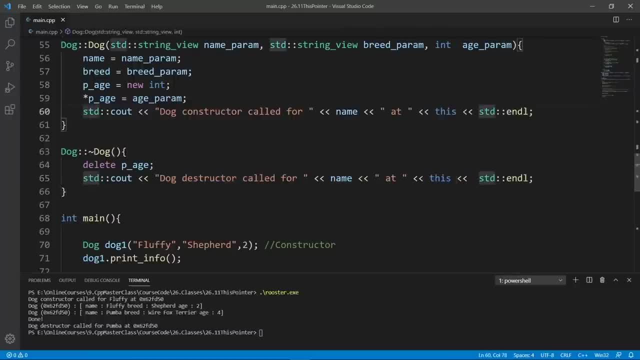 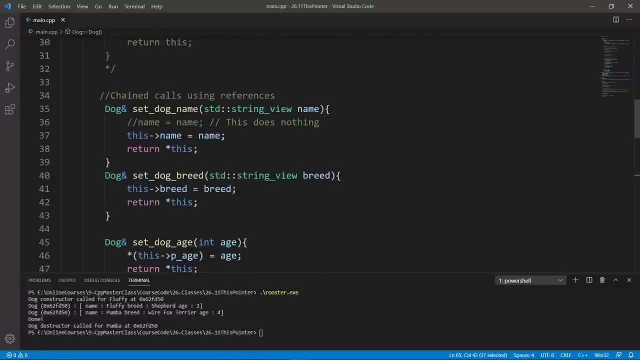 to change the name of our creator to keep the background color blue, and I guess I'm gonna have to stop because we are still waiting for a review, also in the database. but in the database, check out my account illegal. don't forget that I can delete all our 있으면 in this containers. 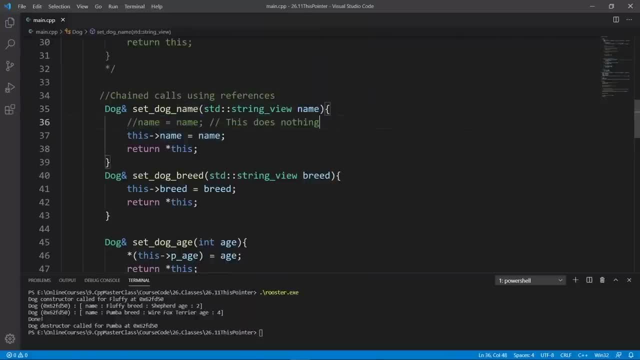 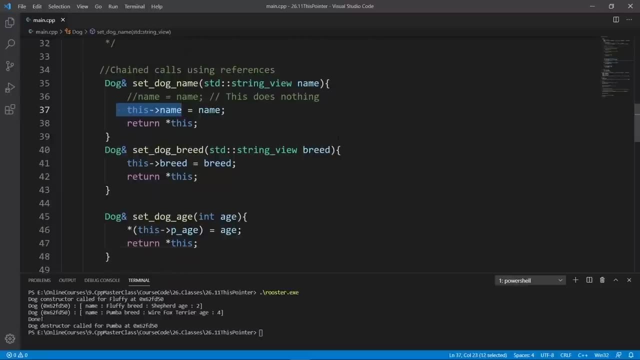 container as well. if we have a way of teams and stubs at all the end users, hard of a job but just to be really confusing and lead to bad results. it's going to change the actual member variable and change it to whatever you pass as the parameter, and this is really cool. we can also 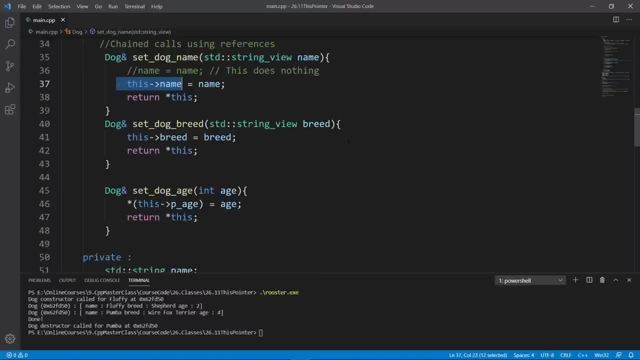 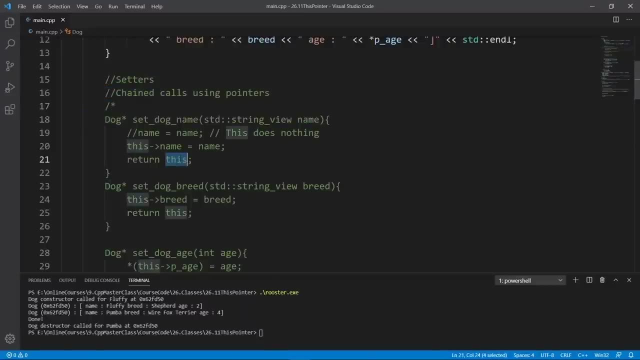 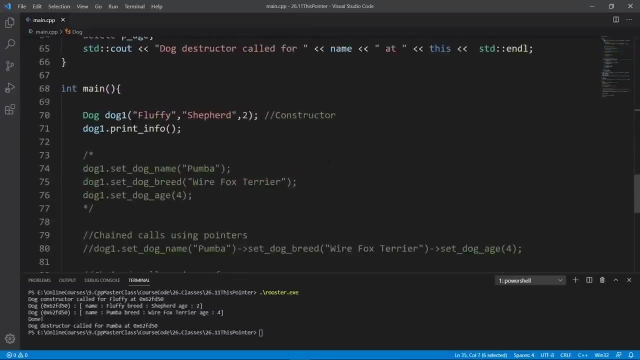 use the this pointer to set up change calls for our function. and we have seen that we can do that either through returning pointers, like we are doing here, and using the this pointer as a return object for our function here, or we can use returned pointers to do this. and if we do that, 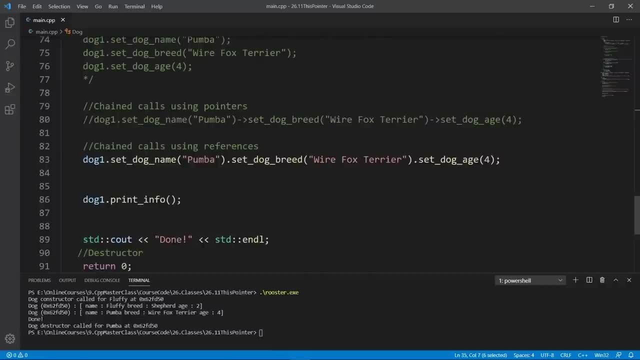 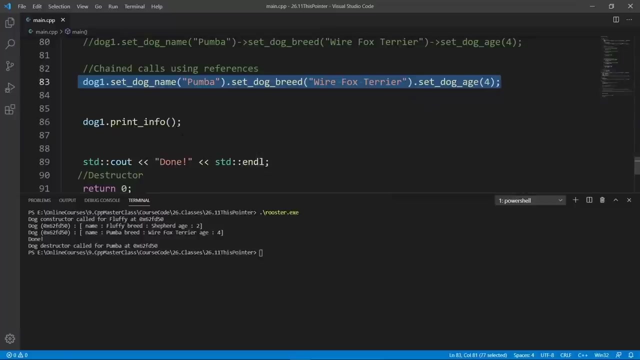 we're going to be able to call our functions in one go, like we are doing here, using pointers, or do the same thing using references, like we are doing here. this is really all we set out to do in this lecture. i hope you found it interesting. we are going to stop here in this one. the next: 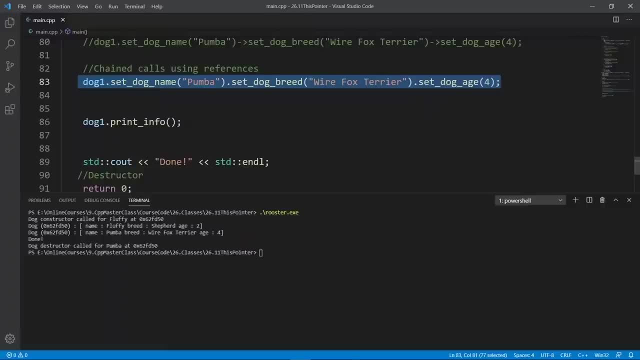 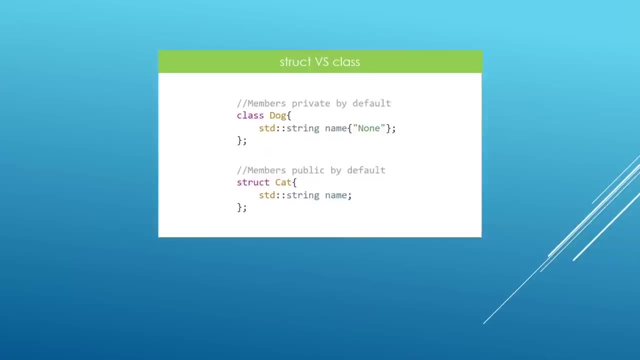 one. we're going to learn about struct. go ahead and finish up here and meet me there. in this lecture we're going to learn about the struct keyword, and this is another syntax you can use to create classes in. I have to break it to you that we can also use struct to do the same, so the syntax here is going. 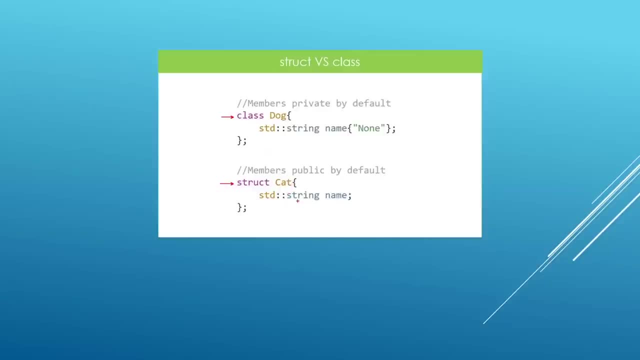 to create a class called cat and it's going to have a member variable called string name. the difference between struct and class is that for classes, members are going to be private by default, and when you do something like this and create class objects, you won't be able to. 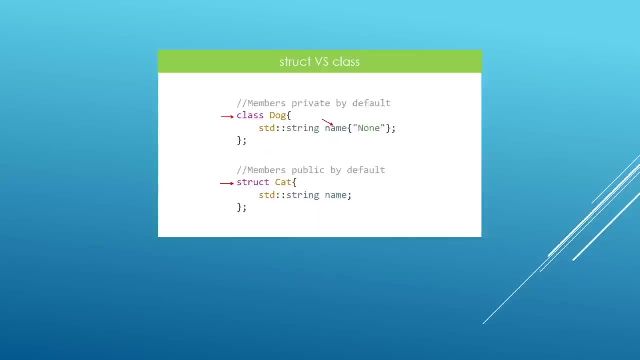 access the name here directly, for example, from the main function. if you do that, you're going to get a compiler error because class members are private by default. but if you use struct, members are going to be public by default and you will have direct access from the outside. this is the only difference. 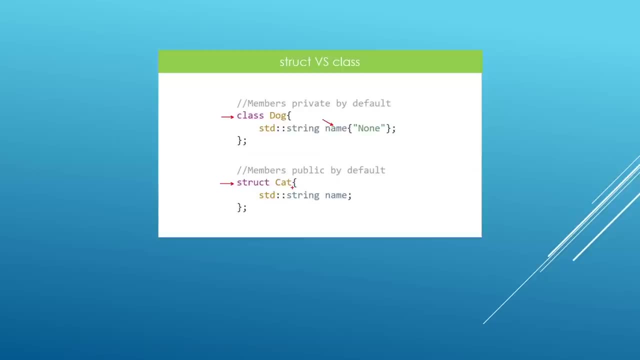 between class and struct. otherwise you can use them interchangeably and they are going to do the same things we have been seeing for classes. they really are the same things. the only difference is that classes are going to have private member variables by default and struct will have public. 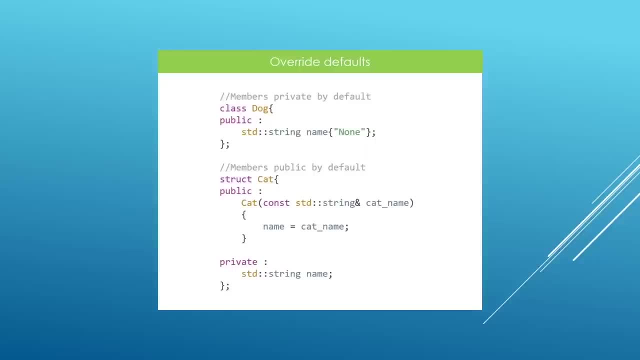 member variables by default, but we can change these defaults by putting in our own public and private sections inside our class. so, for example, here you see that we have changed our dog class to have a public member variable through the public keyword here, and we can do the same for 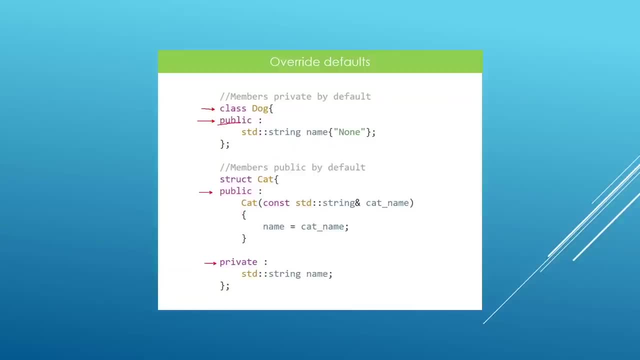 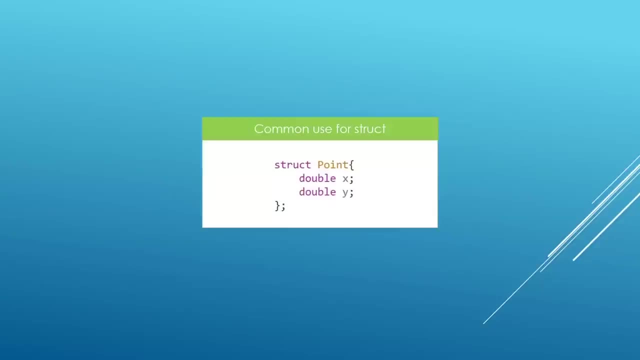 cat, for example. we can put in a public section and a private section and it's going to behave like a class we have been welding so far. one common use we have for struct is when we have to set up classes that only have public member variables. for example, you can need to set up a point model. 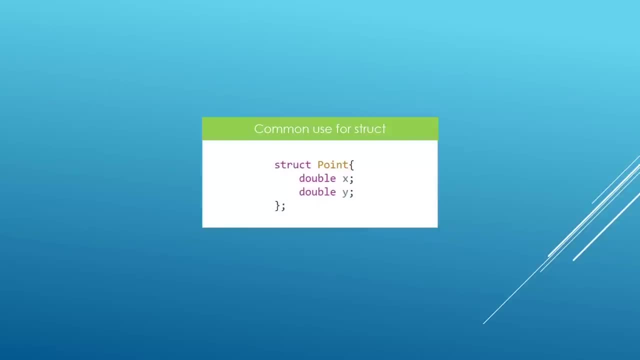 in your c++ program and you can set up a class like this. you can say struct, point. you're going to put in the member variables and they are going to be directly accessible from the outside, and this is something you will see a lot out there. so this is really all about. 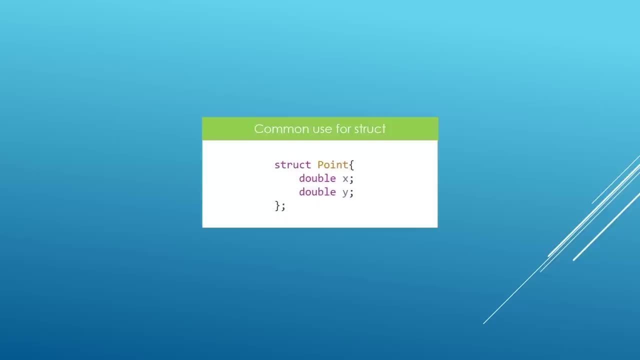 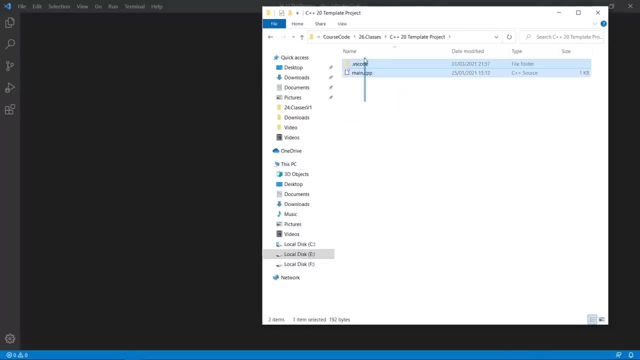 struct. we're going to head over to visual studio code and play with this a little more. okay, here we are in our working folder. the current project is struct. we're going to grab our template files and we're going to put them in place. struct- that's our project here and we're going to open. 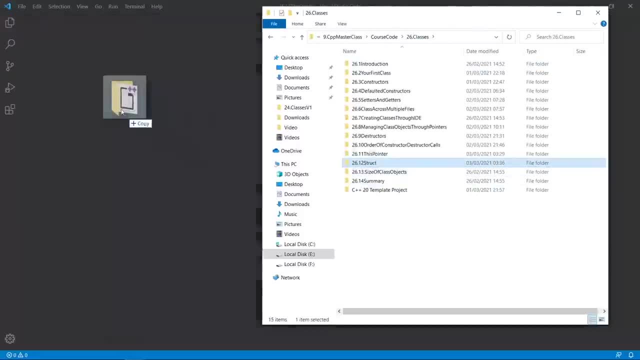 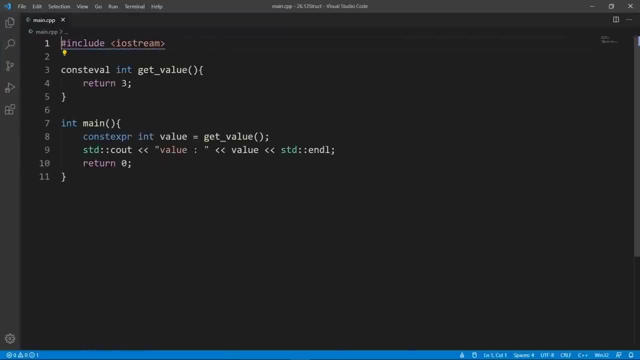 this in visual studio code. let's grab, struct and drag and drop on top of visual studio code here. this is going to open our folder. we can now open the main cpp file and clean things up a little bit. okay, so we're going to set up a simple class called dog. we're going to say class dog and inside. 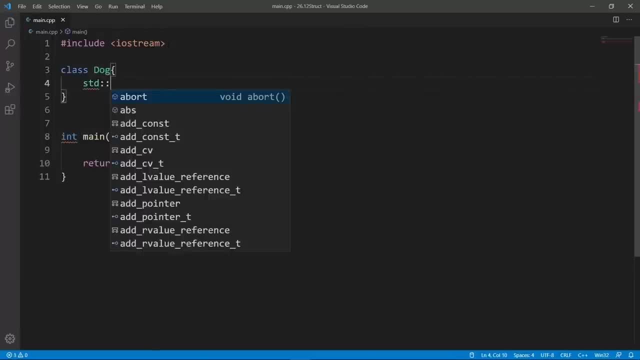 we're going to have a member variable called name. it's going to be an std string. let's say dog name or m name to mean that it is a member variable. this is a syntax. you will see a lot in c++ out there, so let's use this from now on. we're going to say m name and we're going to have another class. 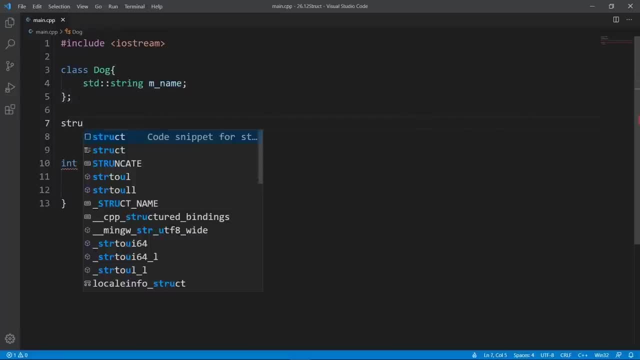 let's put our semicolon. we're going to use struct to set up another one and it's going to be called dog. let's call this cat, and we are going to go inside and set up our member variable. we're going to say std, string, m, name, and it's not going to have anything n. so if we create objects, 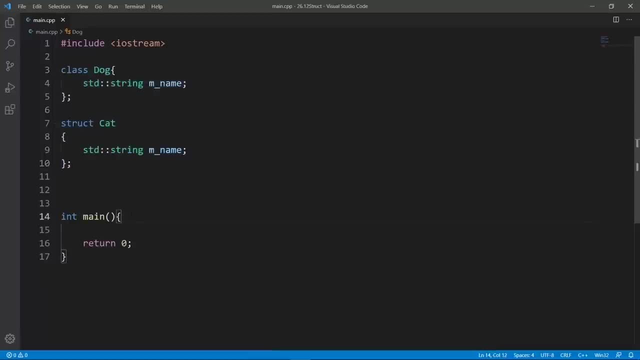 of these classes and try to access them. we're going to see the fundamental difference between struct and dog. let's create a dog and we're going to say dog one. and we're going to create a cat and we're going to say cat one. and if we do dog one and try to access the m name member variable. 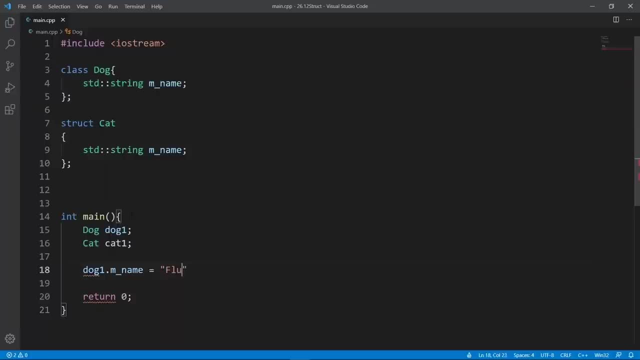 maybe set it to something else. let's say, fluffy, we're going to have a compiler error because members of a class are private by default and we can't really do this. so we are trying to access something that is private from the outside. we're going to get a compiler error. okay, so we have a. 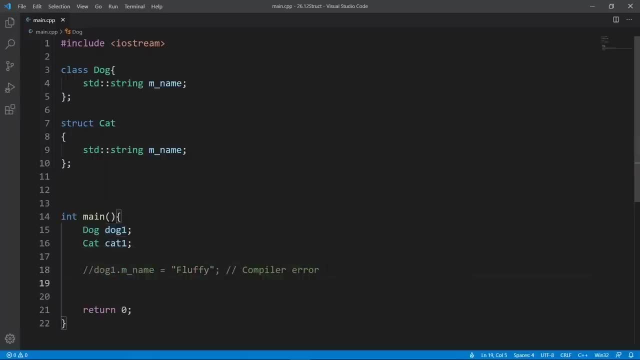 squiggly line here, but if we're trying to do the same for cat, it's going to go through, because cat is a struct and members of structs are public by default. let's do that and really show you this. we're going to say cat one and we're going to say m name and we're going to give it a name and let's say johnny, i am. 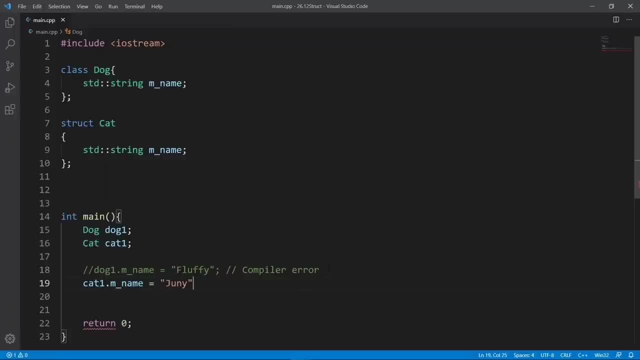 making this up. i don't know if there is any cat named johnny, but we're going to use this and you're going to see that we don't have any squiggly line. we're going to build and see if gcc is going to take this. it's going to take it. the build is good. we can bring up a terminal and run the program. 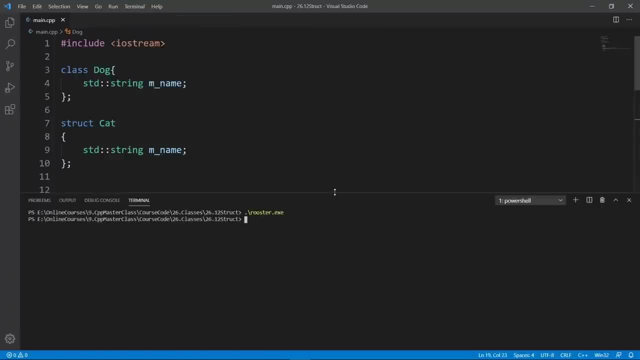 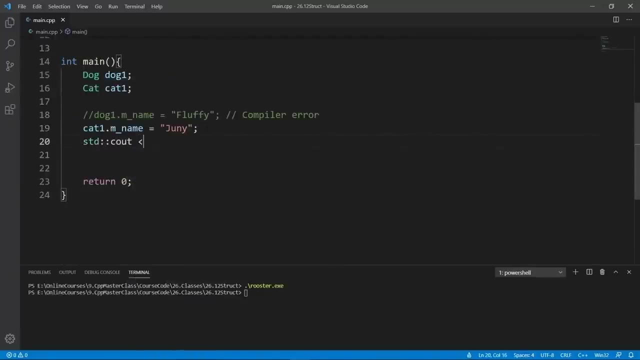 and we're not going to see anything because we're not creating anything from the main function here. but if we want we can print this name of our cat. we're going to say sddc out and say cat, one name. and if we build we're. 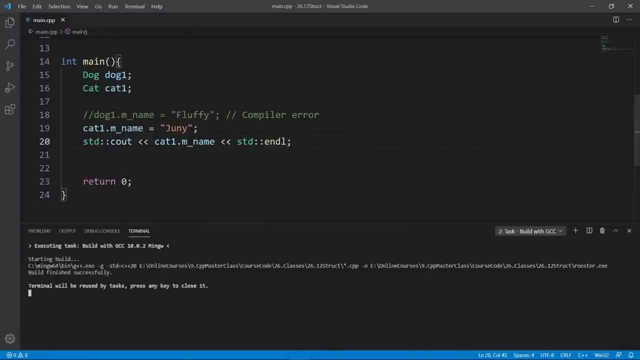 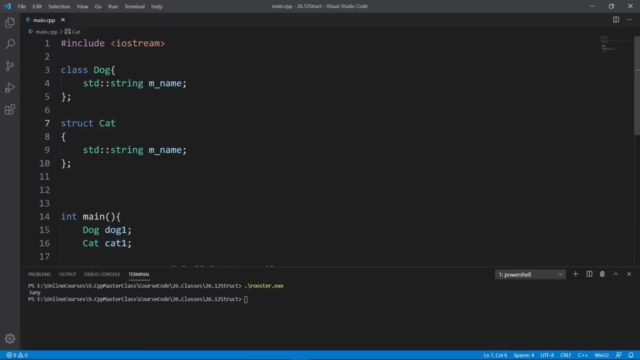 going to see that, so the build should be good. it is good, we can clear and run rooster and we have johnny printed out and this is the name of our cat. and this is really the difference between class and struct. members of classes are going to be private by default. members of struct are going. 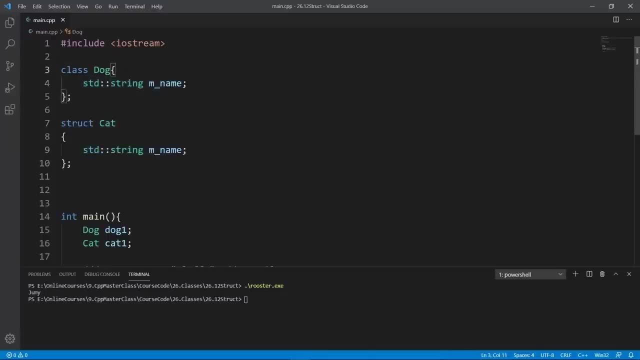 to be public by default, but we can change these defaults. for example, let's make everything public. we can do that no big deal here, and we kind of move this a little bit to the right so that things are aligned nicely, and we can do the same for struct. okay, so let's align this now. if we do this, 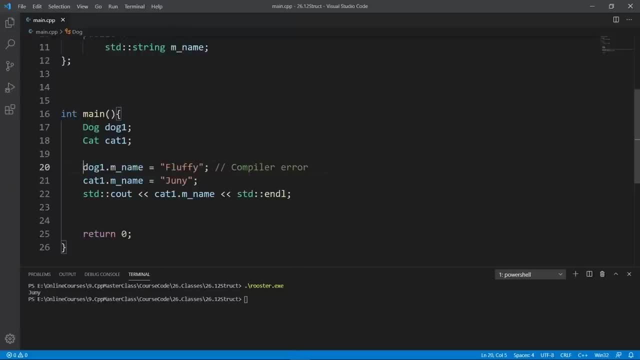 we will be able to go in the main function and say dog name and change that and we're going to be able to see that if we print that out. so let's go down and say sddc out and say dog one name and print that out. and if we're going to print that out, we're going to print that out and we're going to. 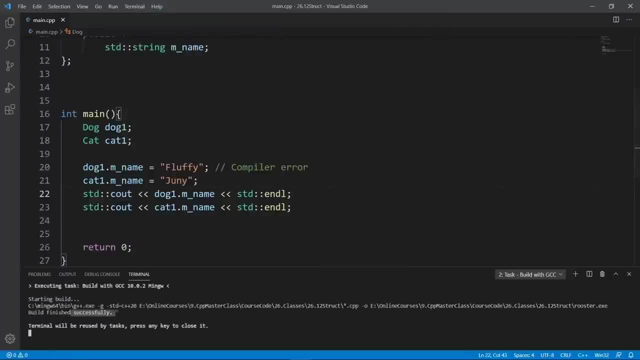 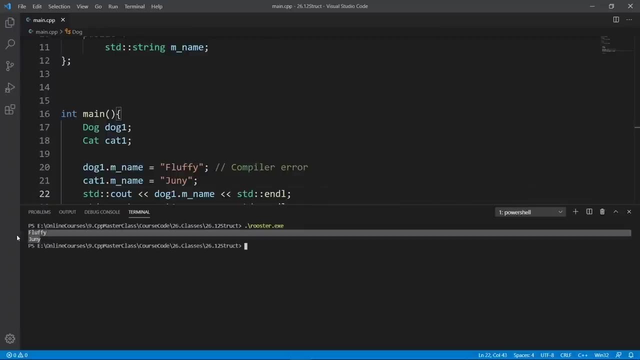 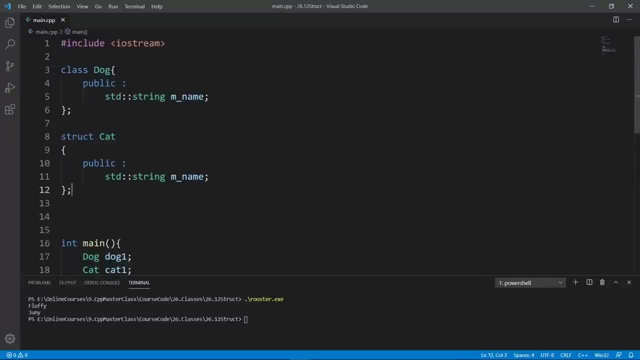 see the name of our dog printed out. okay, build is good, we can bring this up and clear a little bit and run rooster. we're going to see fluffy, our dog name, and johnny, our cat name. so this is really all about classes and struct. they are the same things, but the only difference is the defaults that come. 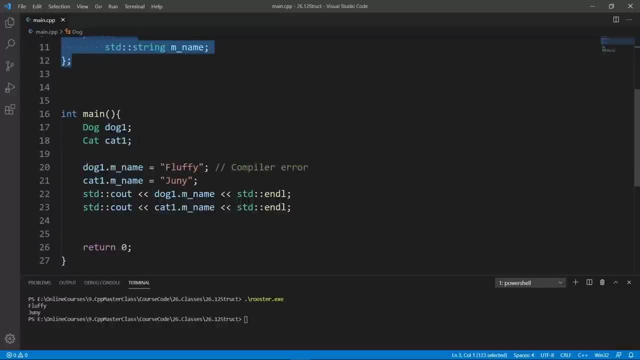 with these things. but the common use we have for struct is when we want to set up a class that only has direct member variables and we don't intend to print out the name of our dog, so we're going to put methods into that class. a good example of this is the struct of point. so suppose we want. 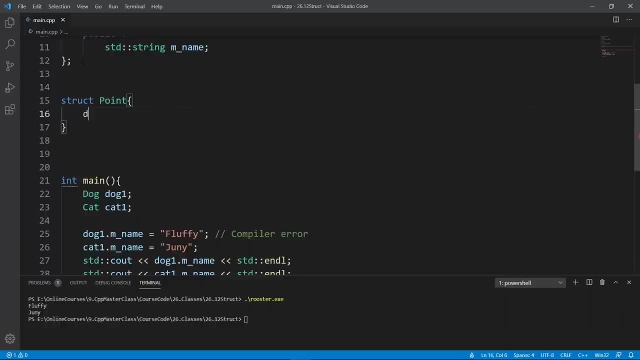 to model points in our c++ program. so we can do something like this: and a point is going to have two coordinates, x and y. we're going to say double y and from this point on we will be able to create point objects and print them out however we want. so, for example, we can go down and say point point. 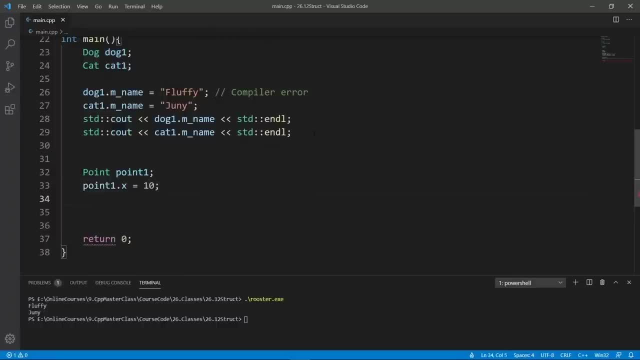 x and assign a value to x. let's put in a 10 and we're going to go down and say point one, y, and we're going to give it a value. let's put in 55.5, why not? and we can do whatever we want with this. 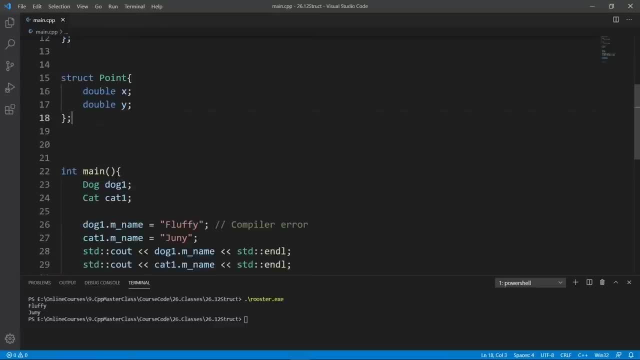 point. for example, we can set up a function which is going to print a point. we can do that, let's say, void print point, and we're going to pass the point by value. or we can even use references, because this is going to be an object cost point reference. i think this is going to do and we're going to go. 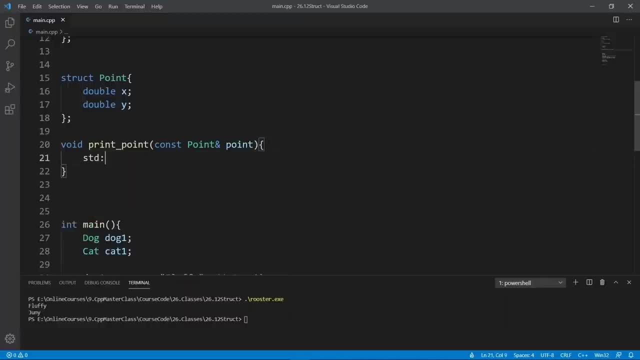 and print the information. we're going to say hddc- out point, and we're going to put the coordinates and we're going to say x is going to be point x and y is going to be point y- why not? and we're going to put in our closing square bracket and we're going to say hddndl to put a new line. 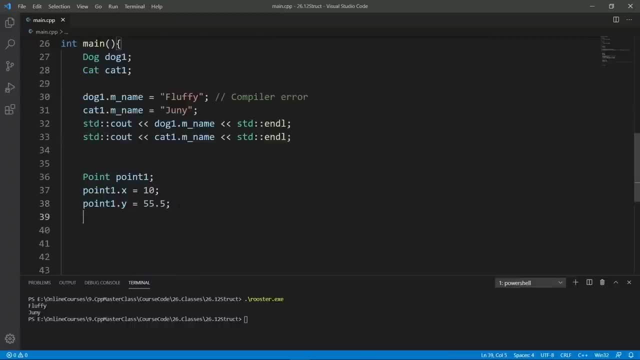 character after our print here. now we can go down and say print point and passing point one, and if we do that we're going to build you and we're going to do that through gcc. you see, the both is good. now, if we print, we should see. 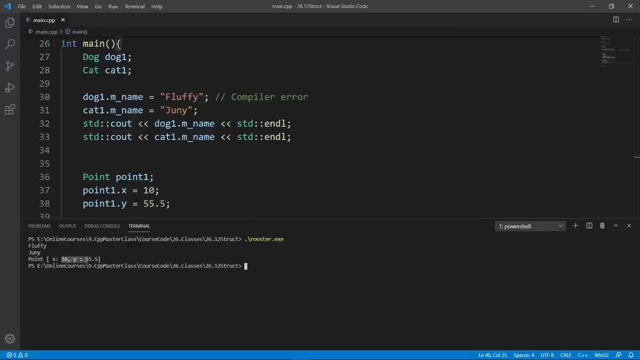 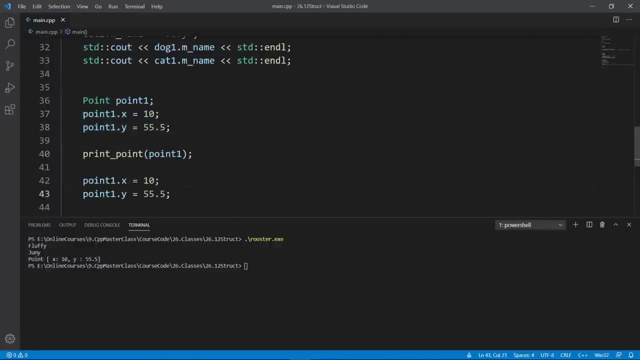 the information about our point and we see point x: 1 y 55.5 and we see point x is 10, y is 55.5. we can go down and change the information about our point. for example, we can copy this and go down and change x to 40.4 and y to 2.5. 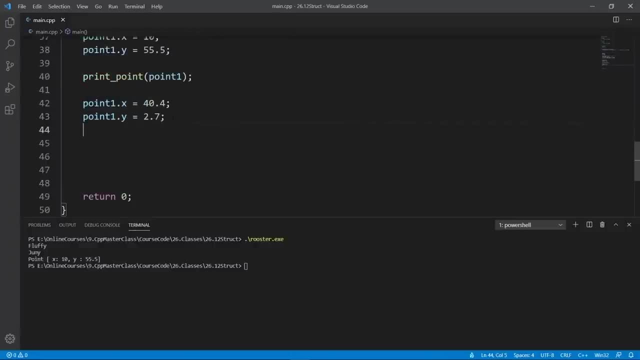 point seven, why not? and if we print the information about our point, we're going to see that we have new information. and we're going to print point one and therefore both. we're going to see the new information, so the both is good. we can clear and run rooster. now you see new. 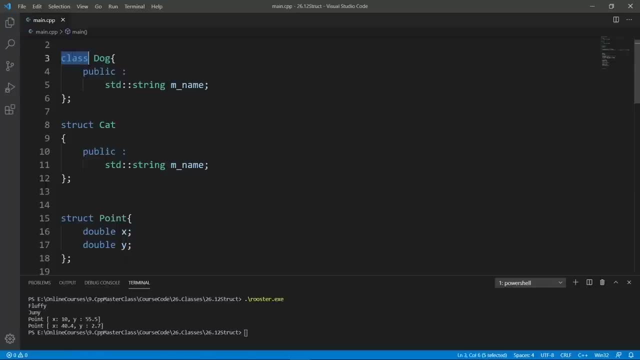 information in our point. so this is really the difference between class and struct. the only difference is going to be in the defaults, and struct is mostly useful if you want to set up classes that only have public member values. you need to make it a feature of the end result and 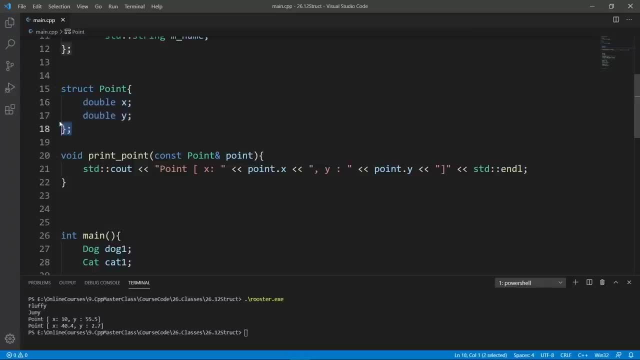 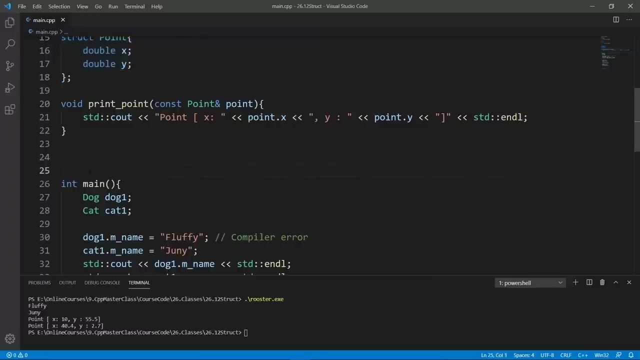 and you don't really want to use functions or methods in that class- and we have an example of that here- and if you have a case like that, you will use struct. your code is going to be much easier to read and understand from the perspective of other c++ developers. we are going to stop here. 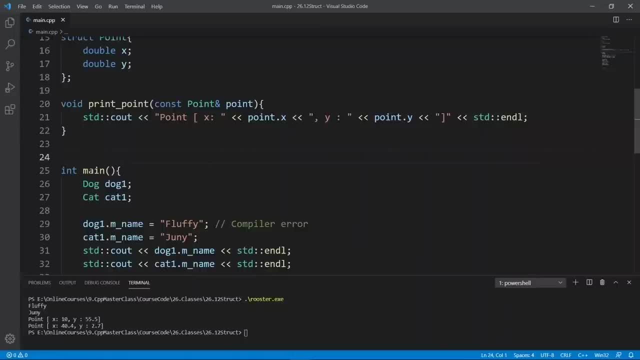 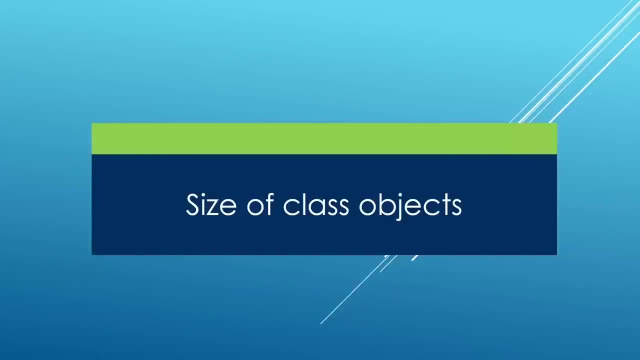 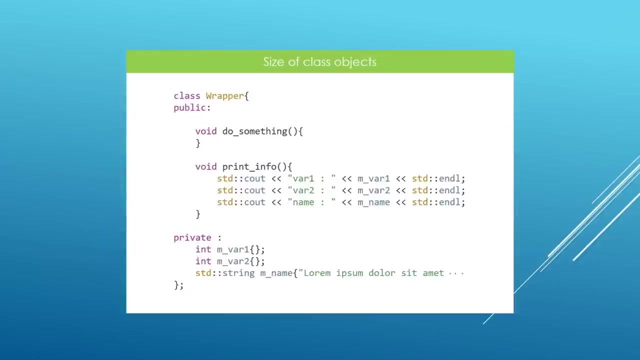 in this lecture. in the next one we're going to learn about the size of objects. go ahead and finish up here and meet me there. in this lecture we're going to learn about sizes of class objects. and try to think about it. what are we going to see if we try to print the size of our class here? 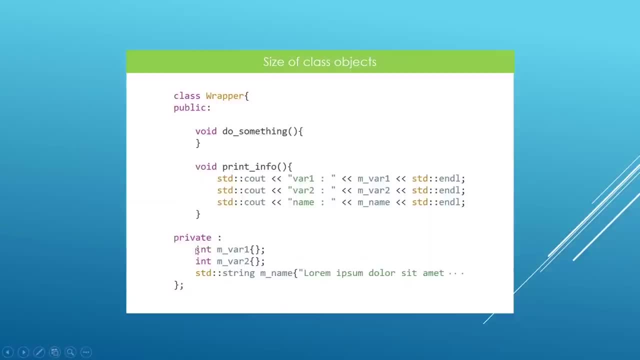 called wrapper. inside we have two member variables which are of int type and we have a member variable which is of std string type. what do you think we'll see when we print the size of this wrapper object here? try to think about it. so what c++ does? it's going to only account for the size of your member. 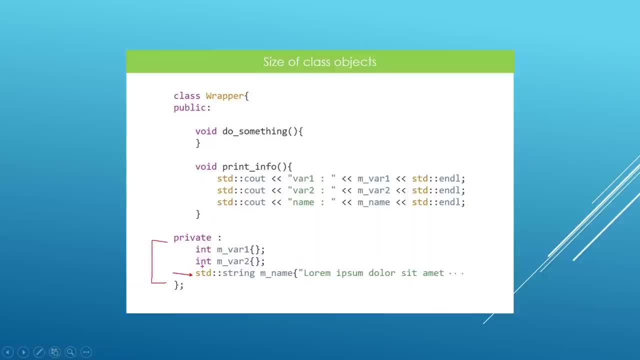 variables. so it's going to add the sizes of these guys in memory. so we know an int is going to take four bytes in memory. so we're going to have eight bytes for these two ints and we're going to have an unspecified amount of memory for a string, because a string is internally implemented as a. 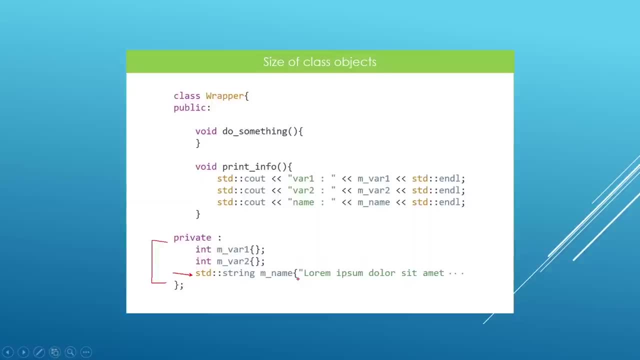 class and it stores its data as const car. so we have really a pointer, and the size of an object doesn't really account for things you are referring to. using pointers, it may count the size of the pointer itself, but it's not going to count what is pointed to. and in the case of string, for example, we really want to know the range of things. 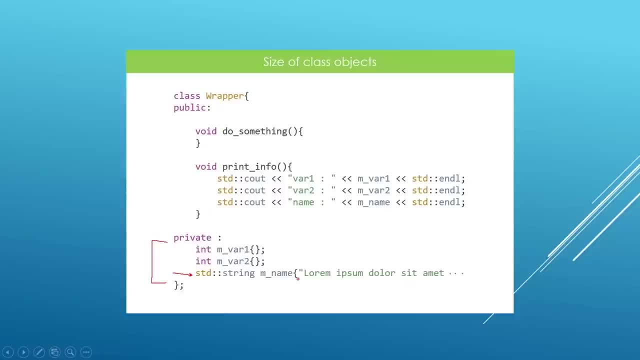 that we are pointing to. so we're not going to have correct information with std string here. but in general the size of an object is going to be the size of the object that we are pointing to be the sum of the sizes of its member variables. the functions are not going to be counted then. 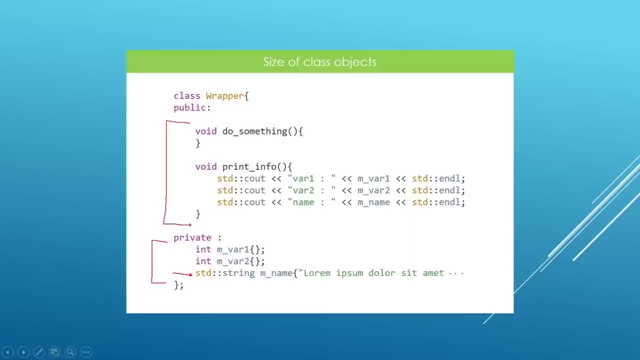 the functions are just helper functions that live somewhere in memory, but they're not going to be accounted for in the size of your object. another reason you might think functions are not accounted for in the size of the object is that really functions are affiliated with the class itself. 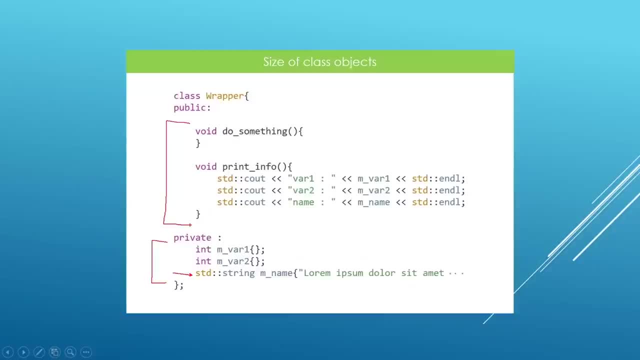 functions are not affiliated with class objects. the class is going to be the blueprint for which we're going to generate thousands of objects if we want, but the functions or the methods are going to be associated to the blueprint itself. so it really wouldn't make sense to associate the 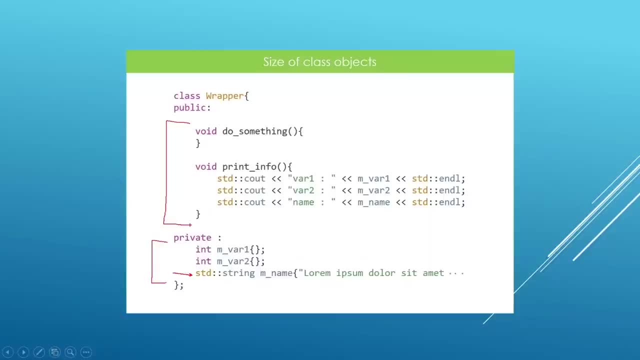 size of those functions in memory to class objects. now that you have this idea, let's head over to visual studio code and play with this a little more. okay, we have said that the size is mostly going to be the sum of the sizes for the member variables, but this is not always correct, because 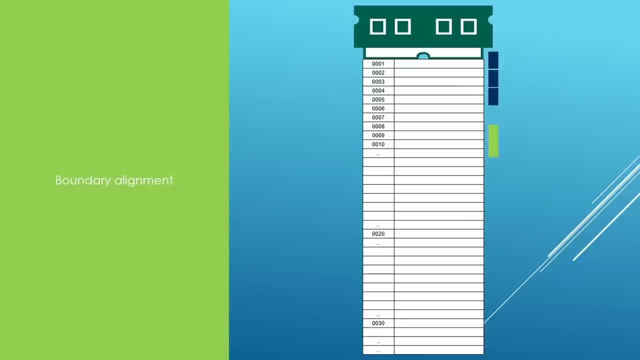 of a phenomenon that we're going to be talking about in the next class, which is the number of variables that are going to be stored in memory, and that is called binary alignment. boundary alignment is a thing most compilers do when they have member variables of different types. 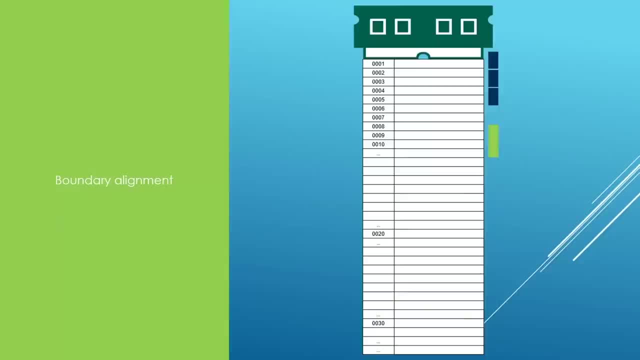 and member variables that have the size of four bytes in memory are going to be stored at memory locations that are multiples of four and because of this phenomenon, we might have gaps between our memory if we have variables, for example, that are of two bytes in memory and four bytes in. 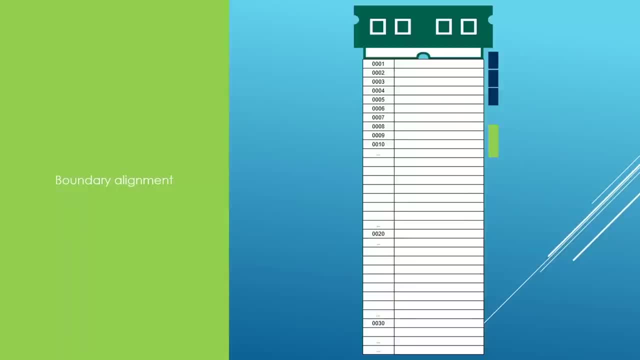 memory and if we have a number of variables that are of two bytes in memory and four bytes in memory, memory and we're going to have gaps inside and the size of the object is going to be slightly off the sum we might do for the sizes of our object. i realize this may be confusing. we're going to 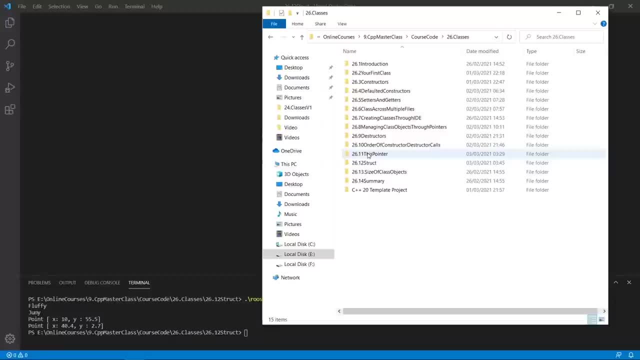 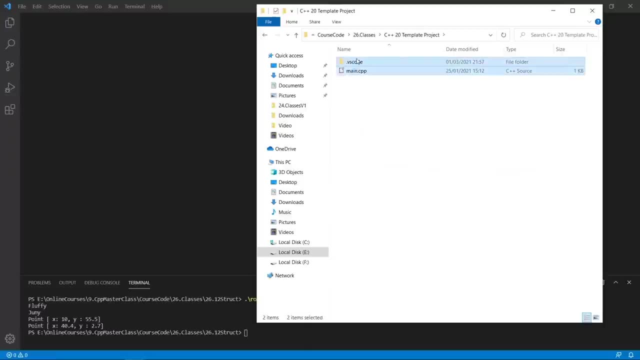 head over to visual studio code and we're going to see a few examples. okay, here we are in our working folder. the current project is size of class objects. we're going to grab our template files pretty quick and we're going to put them in place and we're going to open our 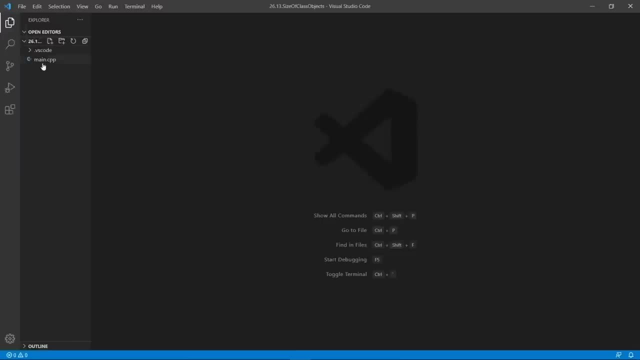 project in visual studio code. by dragging and dropping. here we have our main cpp file. we can close the left sidebar and we can clean the main function. here we're going to set up a simple class. let's call this dog, why not? we have been using dog, so let's use this again. we're going to 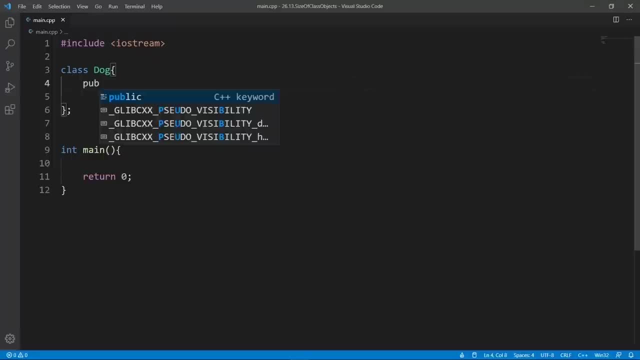 put our closing semicolon. we're going to put a public section and it's going to just contain a constructor and we're going to say dog. and we're going to use the default and we're going to put in a private section and in here we're going to put in a size t and say: this is the leg count of a dog. why not, let's? 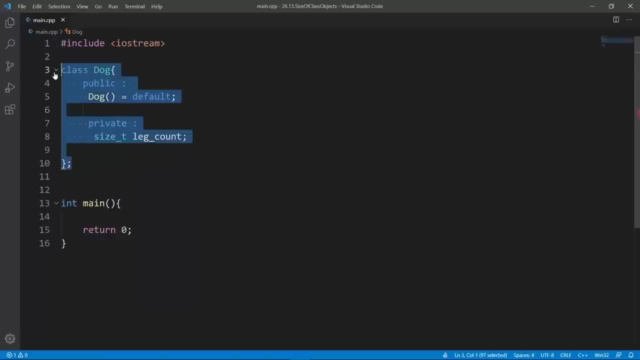 say we are modeling this. okay, so now we have our dog class in place, we can create objects of this dog class. we're going to say dog, dog one, and if we do this we are interested in knowing the size of our dog class here. so we are going to say: stdc out size of dog. you can say that. 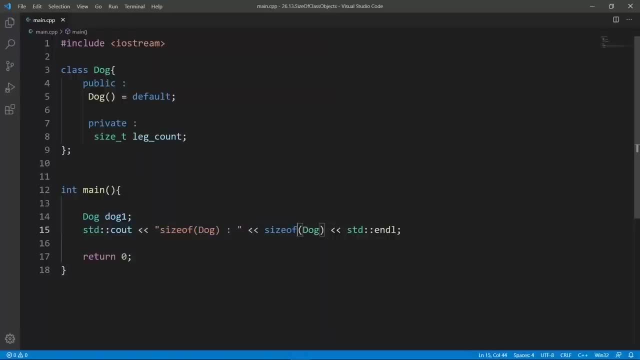 and fingers crossed. we're going to see the size of our dog object here and try to guess what we're going to get in the slides. we have seen that the size is mostly going to be the sum of the size of the member variables. and let's print the size of size t here, because size d is our only member. 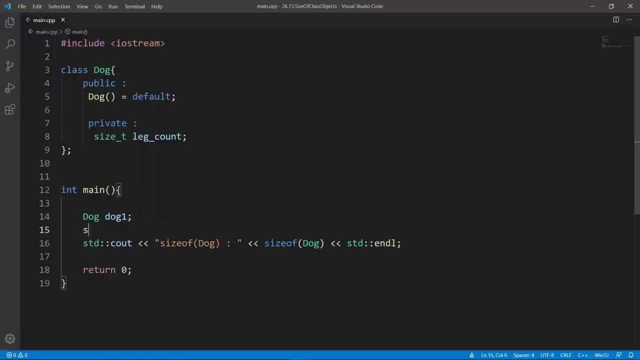 variable, so i think it's going to be helpful to see its size printed out. so we're going to have some context. if we do that, we're going to say size of size t and we're going to say that and we're going to build this program. let's do that. we're. 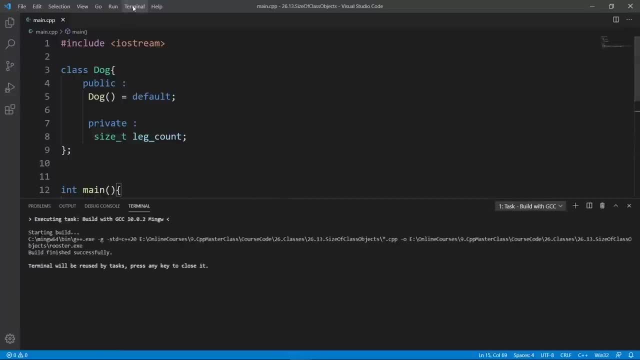 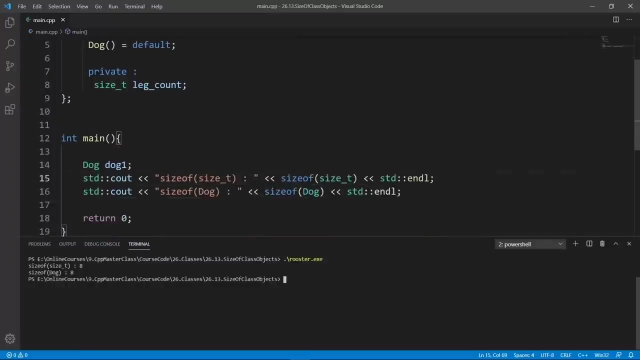 going to pass this through gcc. you see, the both is good and we're going to bring up a terminal and run this. see what happens. okay, we see size of size t is 8 and the size of our dark object is 8, and this is really cool because we see that the size of our class object is. 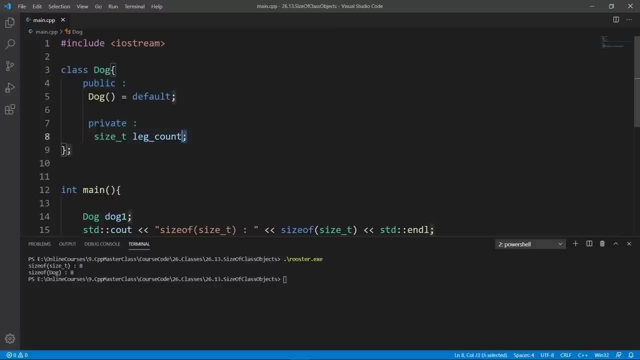 really the size of our member variables that we have in here. let's set up another member variable and really show you this. so we're going to have arm count, okay. so we are just messing with us to learn. i don't aim for this class here to make some sense practically, we just 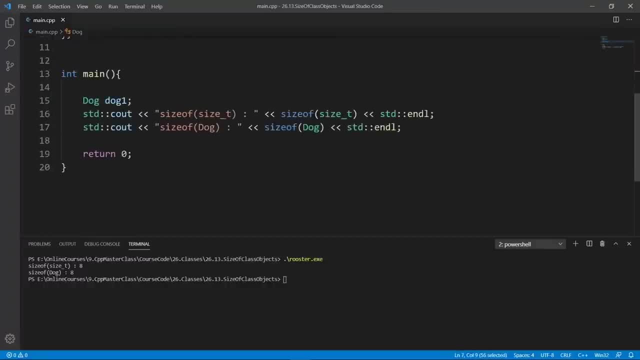 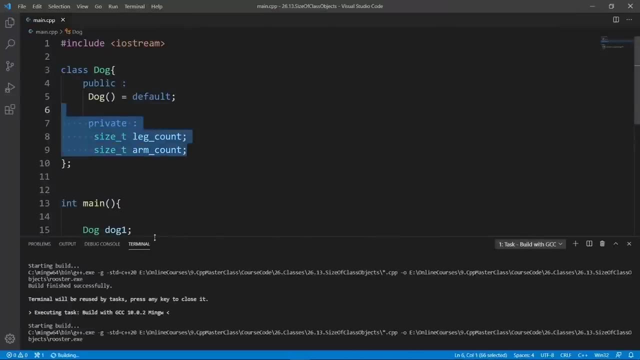 want to see how the member variables affect the size of our class object. now we have two member variables in. we're going to try and weld, we're going to use gcc to do that and we're going to clear and run rooster. now you see, that size of dog is 16 and this is really proving that the size. 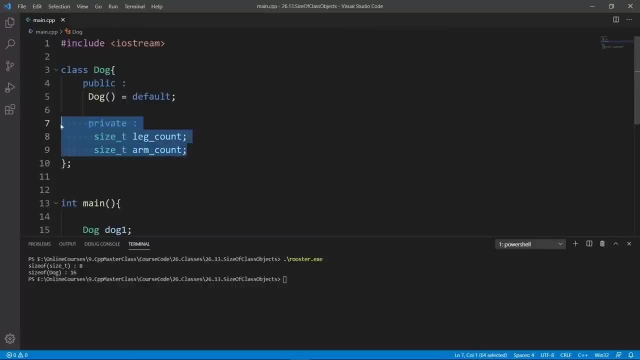 of an object is only accounting for the sizes of the member variables. it's not going to count the functions that we have here. so if, for example, we had a function that says printable and we have another one that says do something, this is not going to change the size of our object because 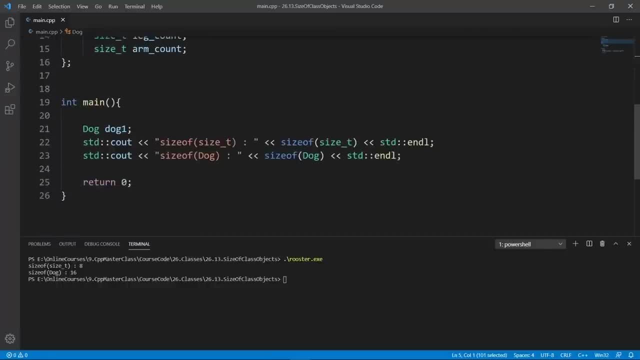 functions aren't accounted for in the size of our object here. so let's build and really show you this. the world is good. we can clear and run rooster. we see that we have the same sizes. the size of dog is 16. the size of size t is 8. we 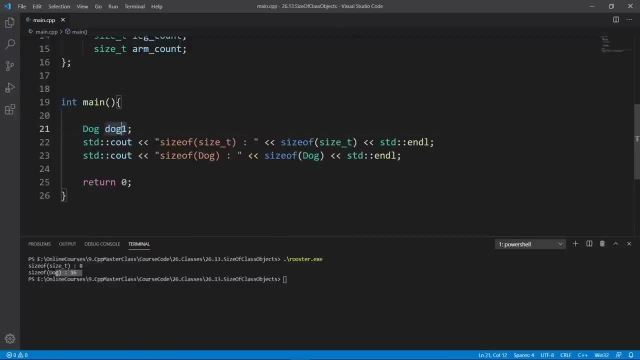 can even use object names. here, for example, we are using the class itself, but we can use dog one here and we're going to get the same information. let's build and we're going to clear and run rooster and you see that we have the same size. so if we 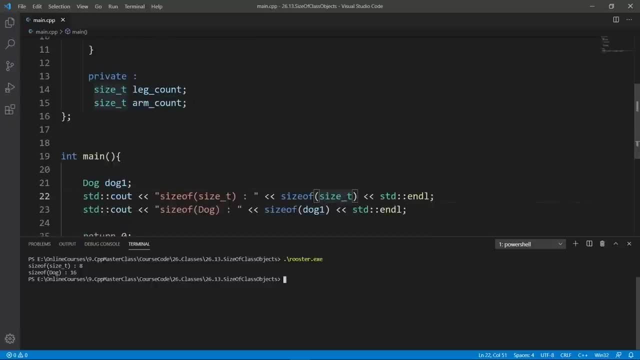 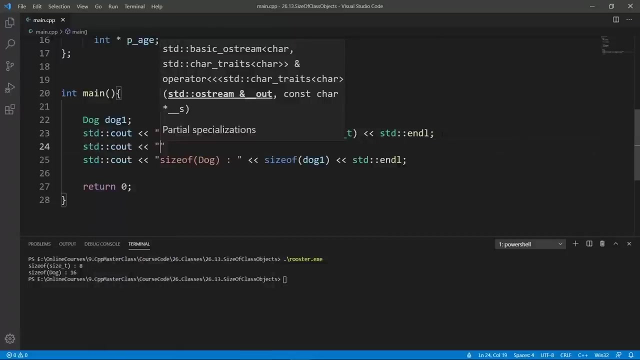 change this thing to put in a pointer, we're going to see something else. let's put in a net pointer and let's say ph, like we have been doing all along, and see what we get. and we know that the size of a pointer on my system. let's print that out so that we have no doubt. let's, for example, say size of. 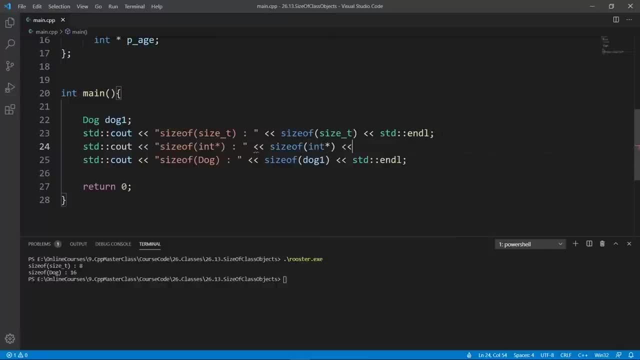 end pointer is going to be size of end pointer. okay, let's build. we're going to pass this through gcc and the world is going to be good. we can clear and run rooster. we're going to see that we have 24 because we have two member variables. that 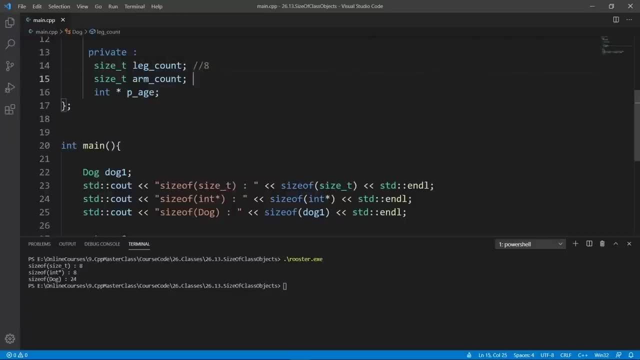 are going to be eight bytes in memory of size t. they are of type size t and we have a pointer which is going to have a size of 18 memory, but we don't care what this pointer is pointing to. if, for example, this pointer is pointing to something really large, we don't care, we're. 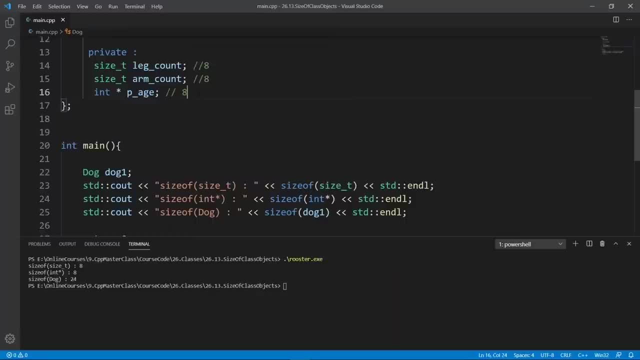 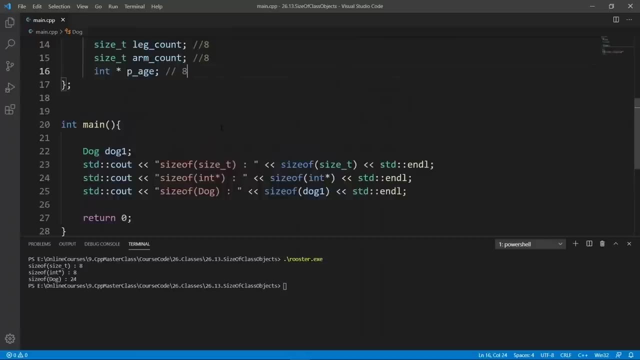 just going to account for the end pointer here. and this is really phenomenal, because if, for example, we try to set up an std string object and by now you should know that std strand itself is implemented as a class in c plus plus, so it's really a class and we can print its size. 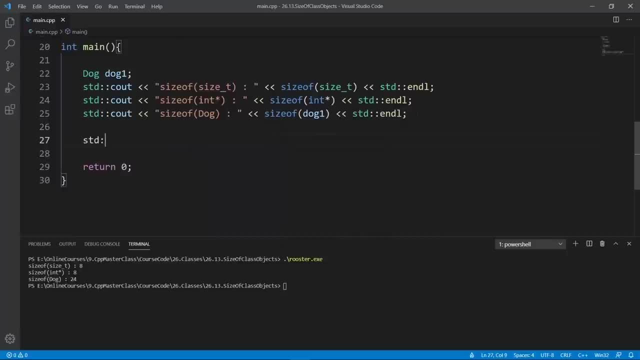 so let's set up a string object. here we're going to say std string and we're going to say name and we're going to initialize this with hello world. okay, we're going to see something really strange here. so if we print the size of name here, we're going to say size of. 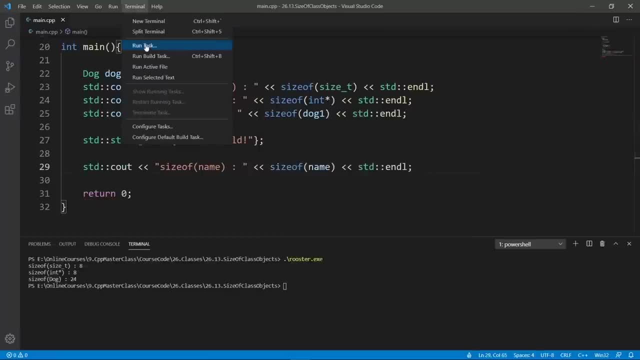 name and we're going to print that. let's see what we get. we're going to run and we're going to see the build is good and it can clear and run roaster. we're going to see that size of name is 32. let's change the text inside our string and see that we change accordingly, because this: 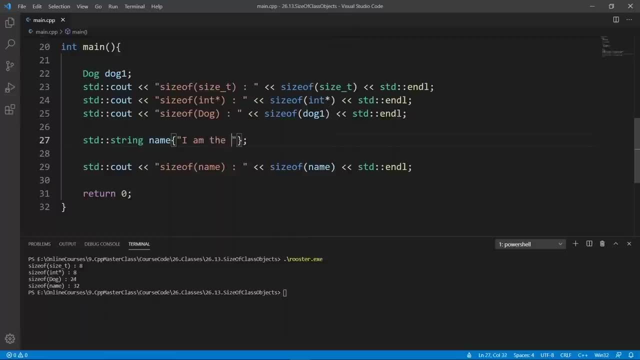 can really be confusing. let's say: i am the king of the universe- why not? and we're going to build again. let's see what we get. fingers crossed. this is going to blow up the string and we're going to see that at the next stage, this point in the string will run like this: this is going to contract. 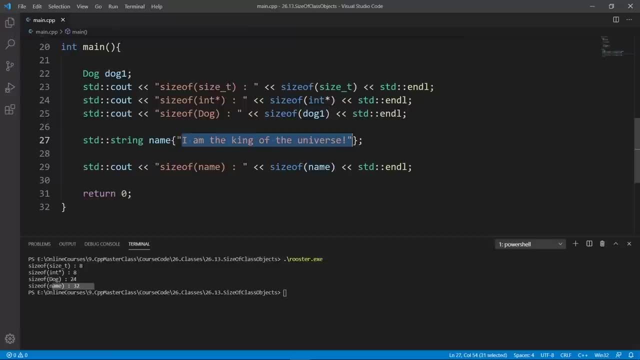 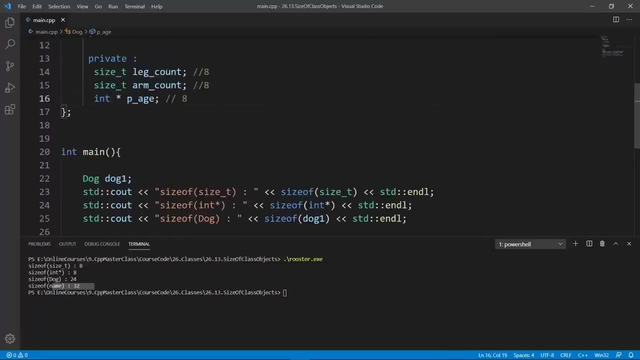 with this and we're going to have the same values. so what the strength is here? it says, let's say, thereib, showing the string- this is the kind of line that you probably notice- is that I actually amайт, which helps me to bullets identify something closer to myory. 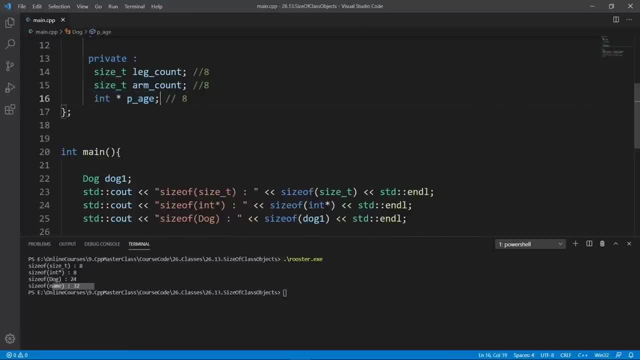 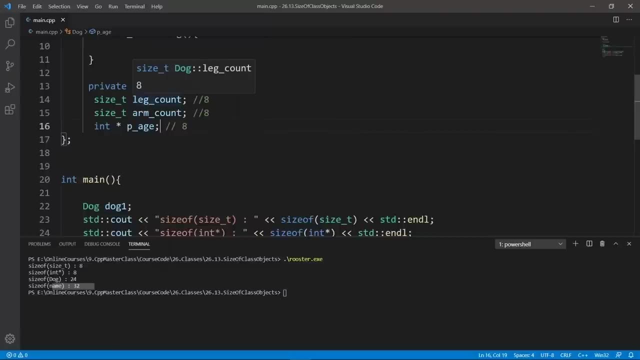 and of course you will recognise when a string occurs. it has been explained. that just means, in part, the size of what is pointed to. okay, so the car pointer may be pointing to thousands of characters in memory, but as long as the compiler is concerned, it's just going to use the pointer. member variable. 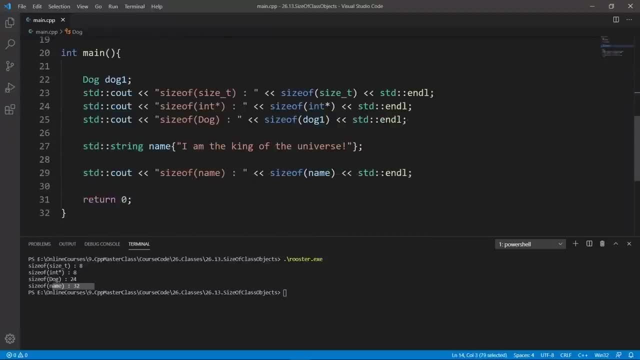 and it's going to account for it in the size of your object. hopefully, you can understand why the size of our string object is going to be the same regardless of how large is the strand, and this is really something you need to understand. otherwise, this is going to throw you off, as you. 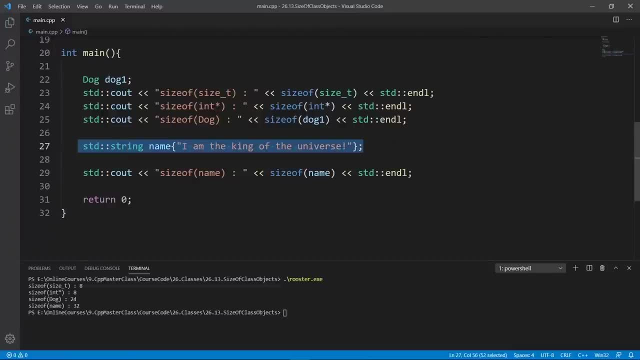 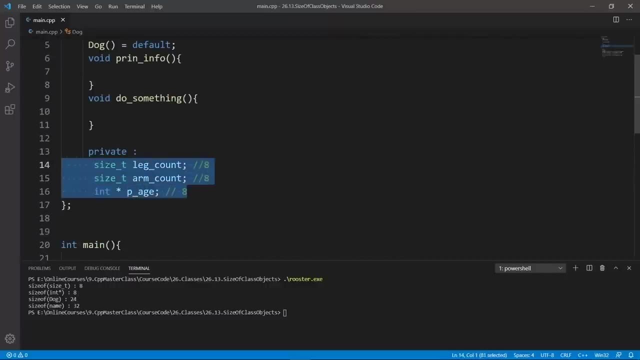 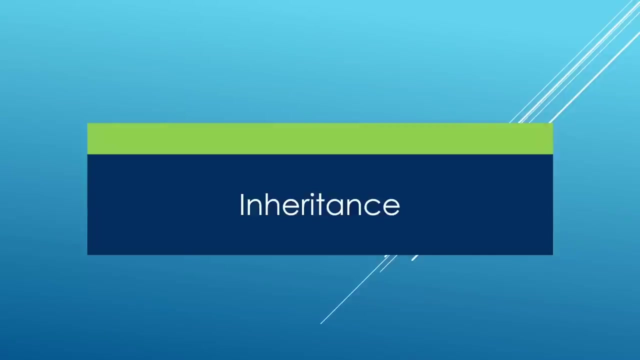 design your c++ applications, and this is really all i had to share in this lecture. the size of your object is mostly going to be determined by the member variables you have, and the size is going to be the sum of the sizes of your member variables. i would like to welcome you in this new 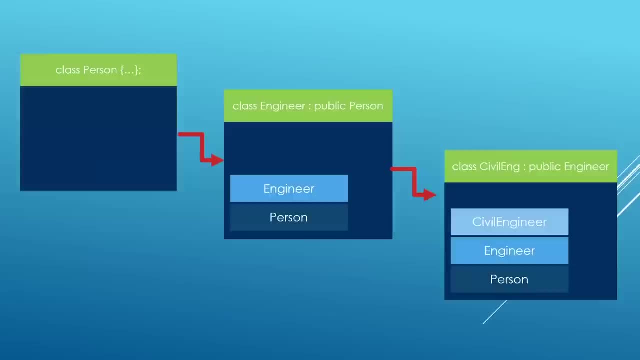 chapter where we're going to be learning about inheritance, and inheritance is a feature that c++ provides to allow us to build classes in terms of other classes, and what i mean here is that we can build complete hierarchies of classes that depend on other classes. for example, if we think of a 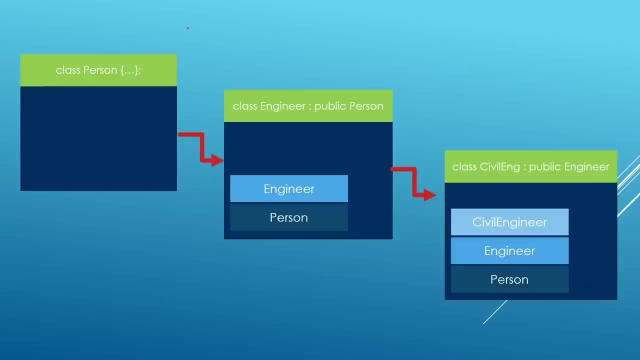 person as a type. we can have different types of persons. we can have a doctor: a doctor is a person. we can have a physician: a physician is a person. we can have an engineer: an engineer is a person. we can have a doctor: a doctor is a person. we can have a physician: a physician is a person. 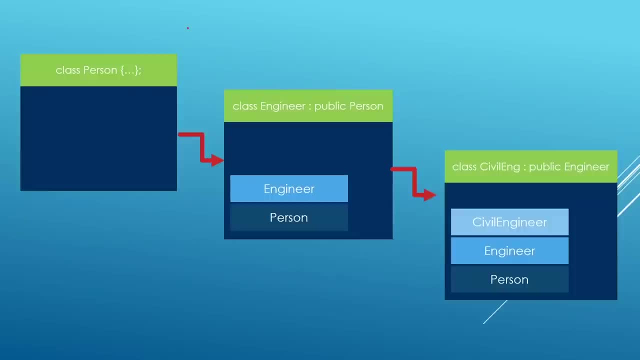 we can have an engineer. an engineer is a person. we can have an engineer. an engineer is a person. we can have all kinds of persons and we can capture these kinds of relationships in c++ using inheritance. here, for example, we have an inheritance hierarchy. we can set up a person type in our c++ program and put in whatever member variables we need to define. 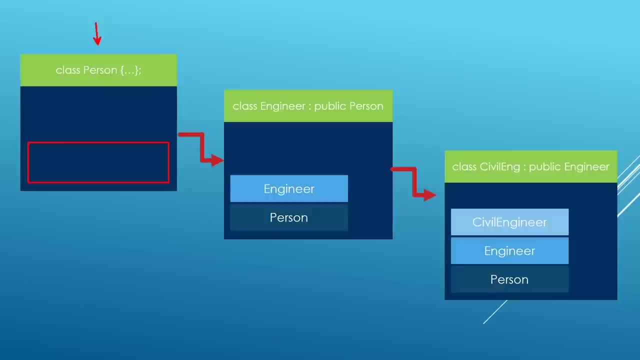 a person, for whatever purposes. we are building our c++ application. for once, we have this type. we can build other types that depend on this person. for example, we can build an engineer type, which is really going to embody the person type inside. so what we will be doing is really: 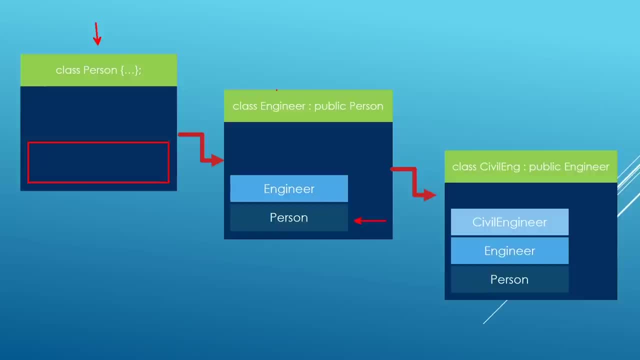 setting up a layer of a person type and in our engineer type, which is going to depend on person, we will build another layer on top of that and really reuse that person type without having to rebuild this from scratch. hopefully you can see that this is going to improve code reuse we can. 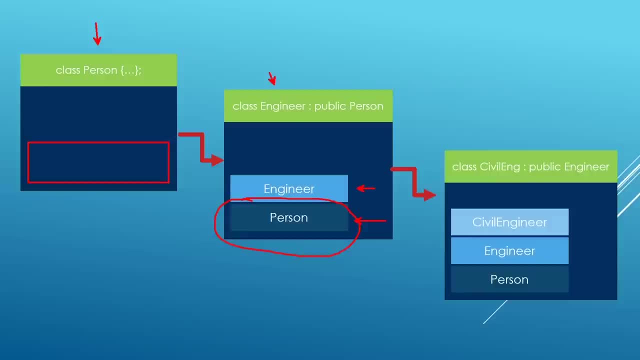 also reuse this engineer type and build other types on top of it. for example, we can have a civil engineer, we can have an electrical engineer, we can have all kinds of crazy engineers modeled in our c++ program using inheritance, and this is going to be really cool. so this is what we are. 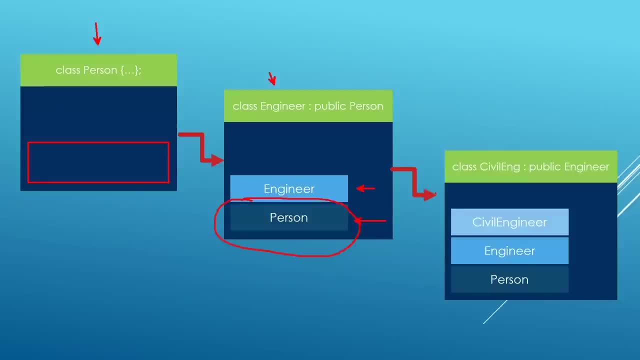 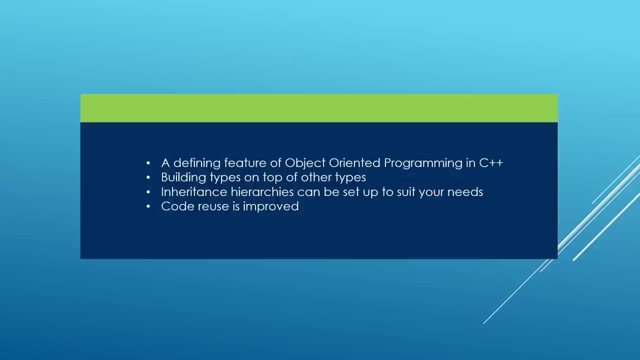 going to be exploring in this chapter, looking at the facilities that c++ provides to capture these kinds of relationships in our c++ programs. please note that, inherently, inheritance is a really big feature and it is a defining feature of object-oriented programming in c++. object-oriented programming is a paradigm or a way of thinking about programming that uses 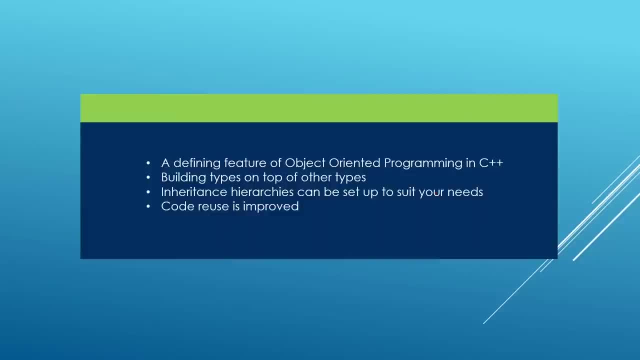 objects and the most basic defining feature of object-oriented programming in c++ is classes. that we have learned about. using classes, we can define things. for example, we can set up a car, we can set up a house, we can set up a spaceship. we can set up a car, we can set up a house, we can set up a spaceship. we can set up a spaceship. 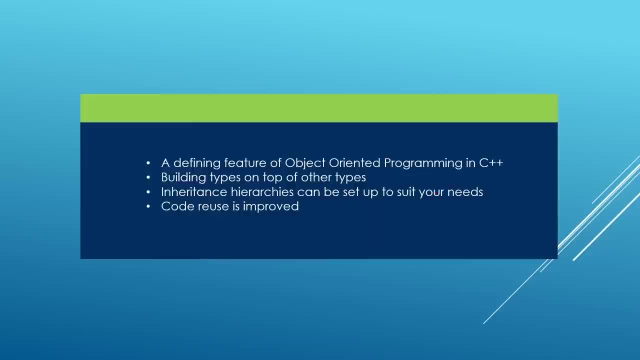 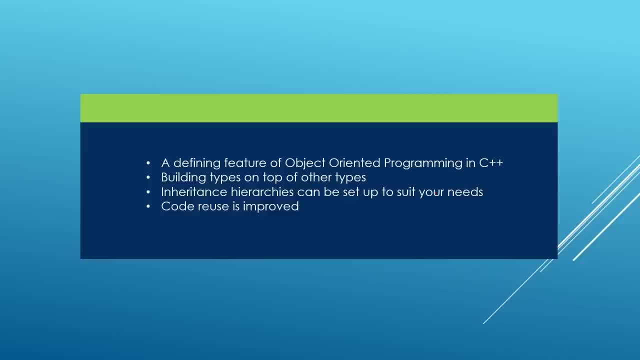 hierarchies that are going to make our design much easier to look at and understand and work with. okay, so this is what we are up against in this chapter: learning about inheritance and really exposing you to as much as possible to let you use inheritance in an easy way. so let's get started. 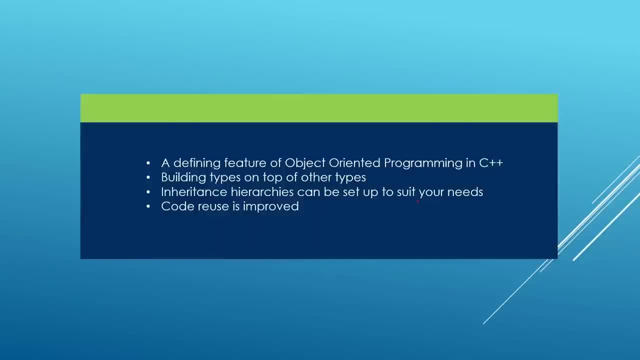 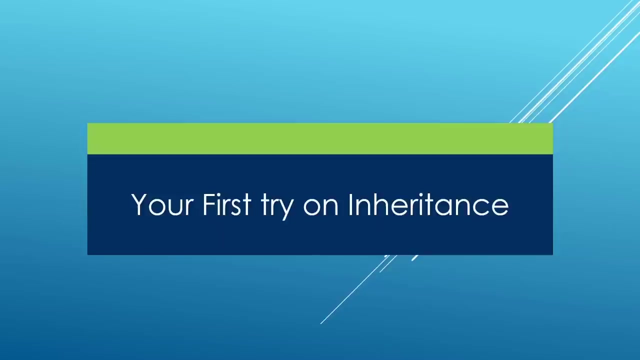 so let's get started in your c++ programs. we are going to start in the next lecture and try out inheritance for the first time. go ahead and finish up here and meet me there. in this lecture we're going to try out inheritance for the first time in this course, but before we do that, let's remind ourselves of what inheritance. 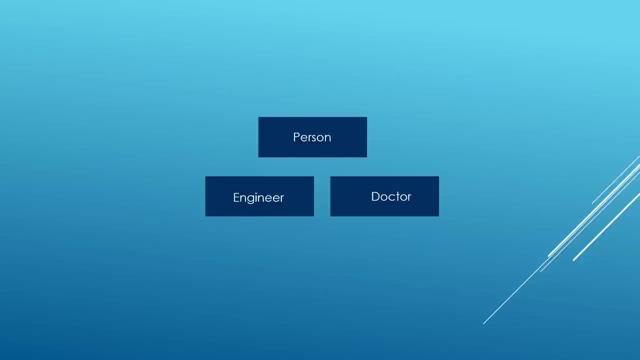 really is. inheritance is a feature we have in c++ to be able to build new classes in terms of the classes we have in c++ and we're going to talk about inheritance in this course and we're going to have predefined and the new classes are going to be stealing features from the already pre-existing. 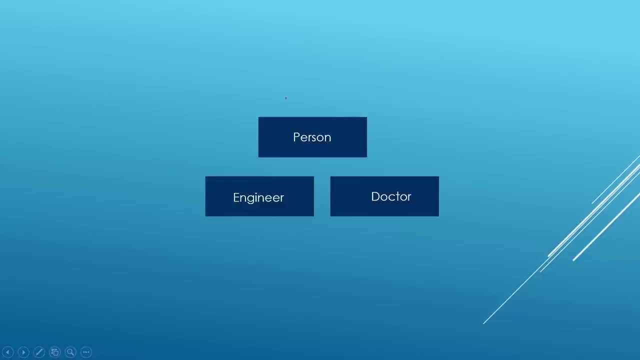 classes, if i can say it like that, and the more classes we build in terms of others, we're going to end up with what we call an inheritance tree, which is basically going to go from the top to the bottom, with the most fundamental class on top and the derived class at the bottom. here we have a 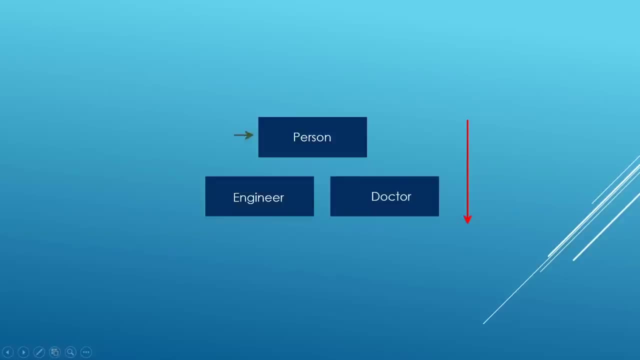 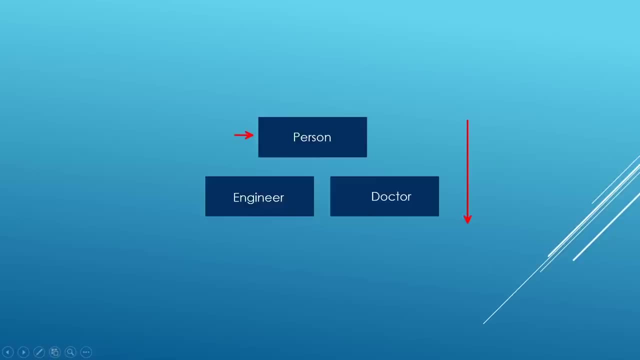 person. but based on that personal class, we might want to derive other classes that build on top of this person class. for example, we might want to define an engineer and a doctor, and we know that an engineer is also a person. so they are going to inherit some features from the person class. 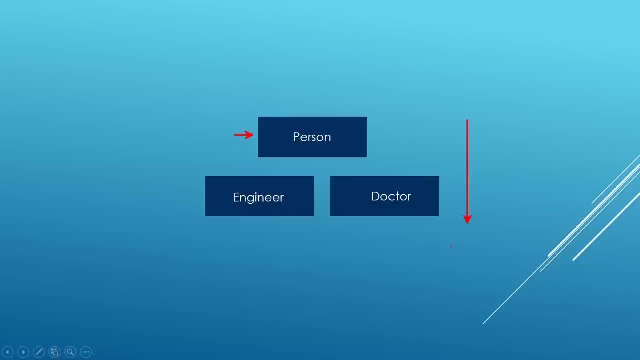 the same goes for the doctor class. it is going to inherit some features from person, but all these derived classes are also going to add their own features to the person. class c plus plus allows us to build these kinds of relationships. here is another simple example. we have a vehicle class to the top of our inheritance hierarchy and below this class. 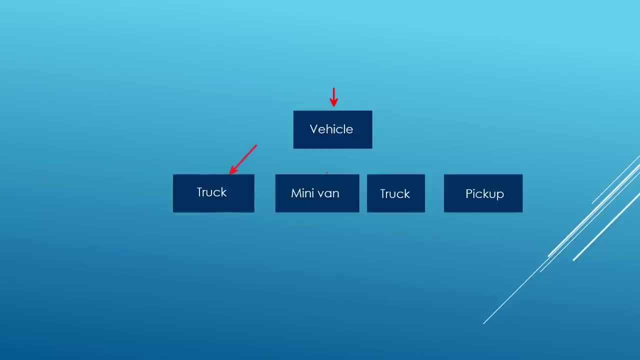 we might derive a track class, which is also a vehicle. we might have a minivan, we might have a truck, we might have a pickup truck. we may really do all kinds of crazy vehicles which are going to inherit the basic features from the vehicle class and add their own specialization. 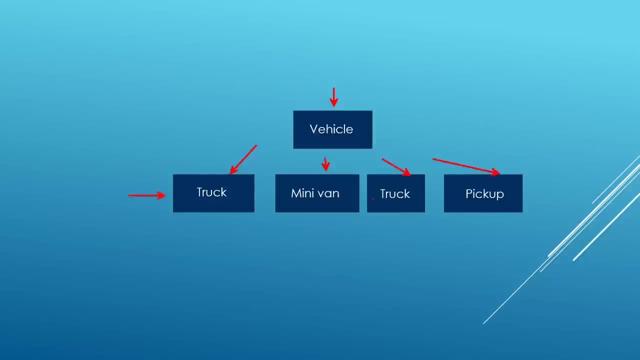 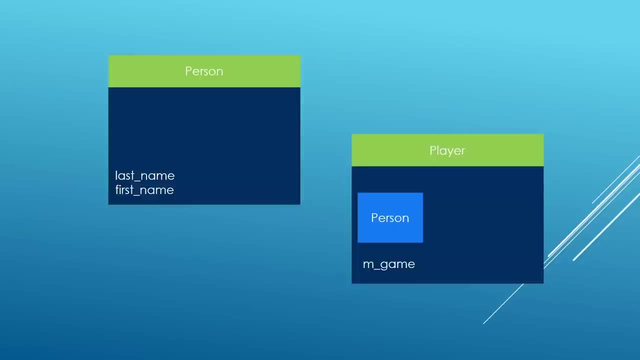 on top of the vehicle class. so this is the basic idea behind inheritance in c plus plus. so the examples we're going to do in this lecture. so here is a simple example of what we're going to do in this lecture. we're going to set up a person class, which is going to be our. 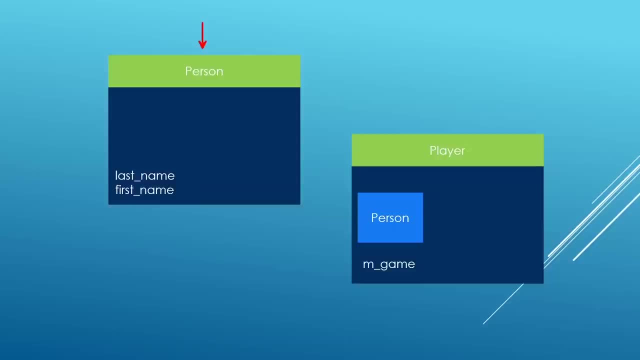 base class. it is going to be defining two member variables which are going to be of std string type. we're going to have a last name for the person and the first name for the person. we are going to derive from this class and set up a player class. 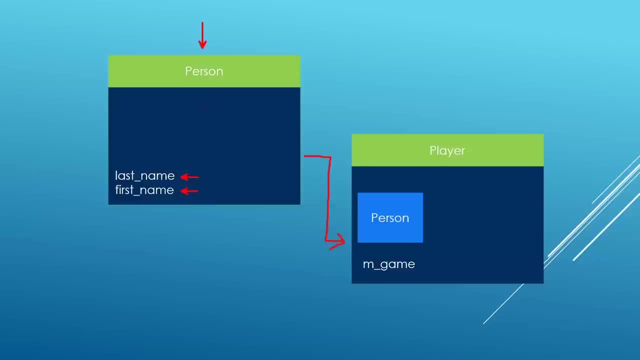 the player class is going to inherit these features from the person class, so it is going to have a last name and a first name built into it. but that's going to be our base or our starting point. we are going to add to this base and add another member variable from player and we're 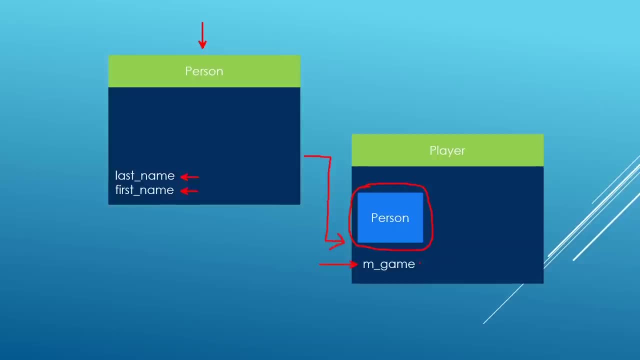 going to be having a player class which is really a person, but it is going to add things to person to customize on what we can do with the player that we wouldn't originally be able to do or have with a person class. this is the basic idea. okay, now that we know this, we're going to set up our 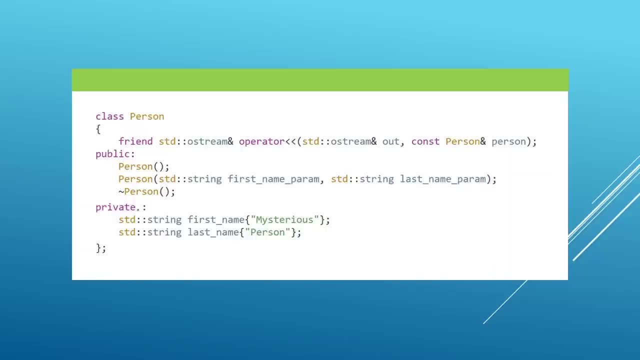 personal class, which is going to be our base class, is going to have our two member variables: first name and last name. we're going to have a bunch of constructors and we're going to have a stream output operator to be able to print this on the console and see our information here. nothing special, but now that this class is done we can. 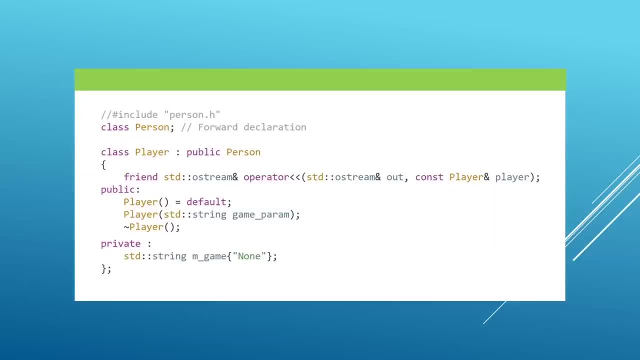 build other classes on top of this class. so what we can do, for example, we can derive a player class. so the syntax is what you see here: we say class player, we say colon, colon, and then we say public and specify the class that we are inheriting from, so the parent class, for this: 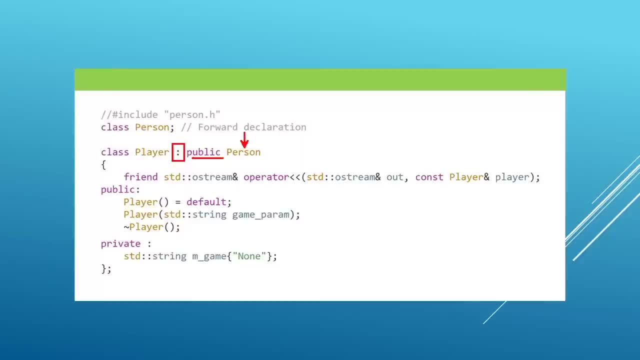 class is going to be person, or in other words, we're going to be deriving from the person class and we're going to be doing that publicly. okay, for now i don't want you to worry too much about this public keyword. we're going to be learning this in steps. 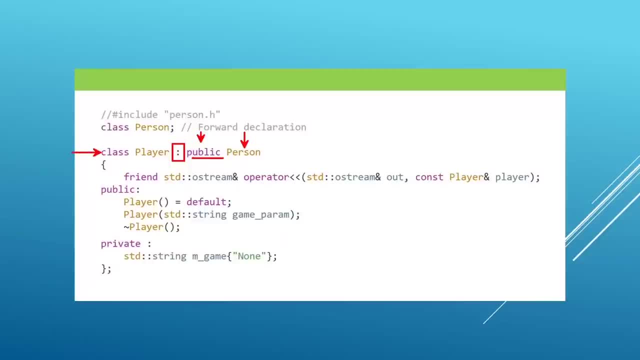 just know that this is the syntax you use to derive from another class. now, the moment we do this, the player class is going to have the personal information embedded inside, but we will also have the ability to customize or add other things at the level of the player class. 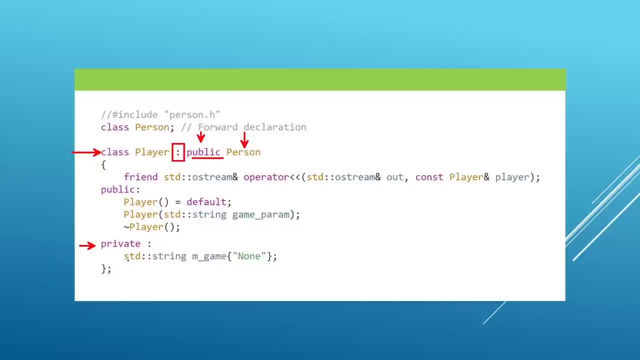 this is what we do. we have a private member variable and it is going to specify the game that the player plays. we're going to have our own set of constructors with us. we're going to have our own set of constructors with us. we're going to have our own set of constructors with us. 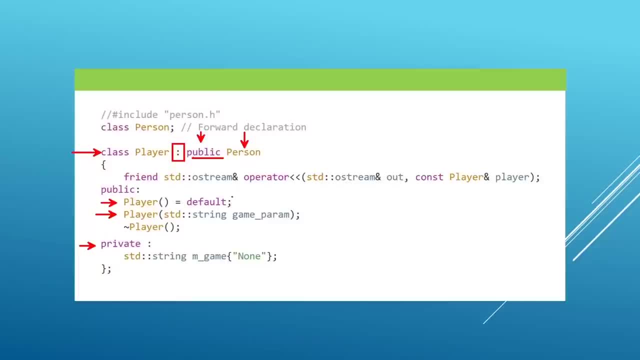 can really build player objects, but they are going to have a person part inside that is going to store information about this player person. you notice we don't have a member variable here for the first name, we don't have a member variable here for the last name, but that information is. 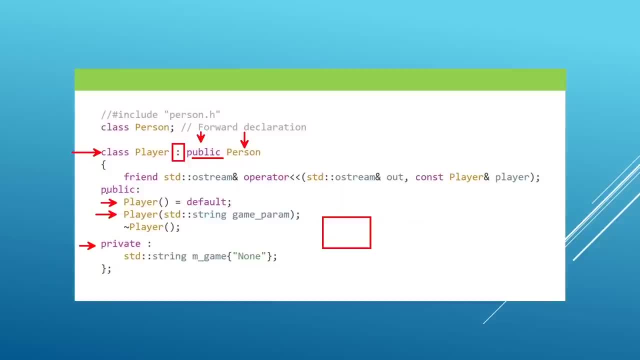 going to be baked into this player object, and this is really how inheritance helps us out. we can derive from classes and build on top of them without having to redo the fundamental work to build our base classes. we can just build on top of them and really do things faster and more. 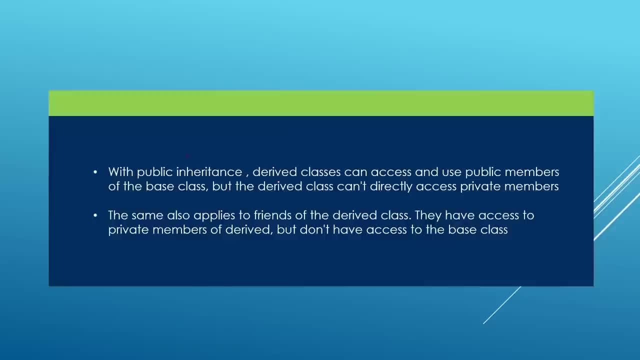 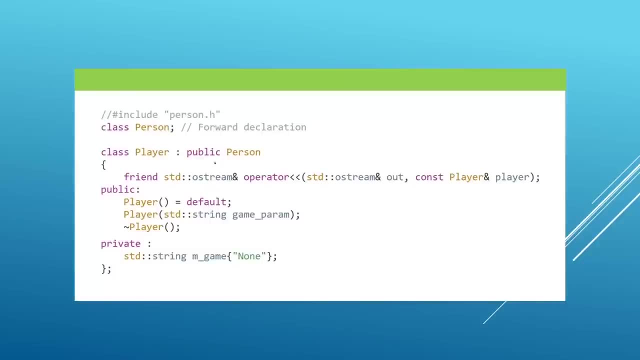 efficiently okay. so here are a few things you need to know about the public inheritance that we just did, and we are saying public inheritance because of the syntax we used here: public person. this is doing public inheritance and we're not just saying through names and by itself, but also 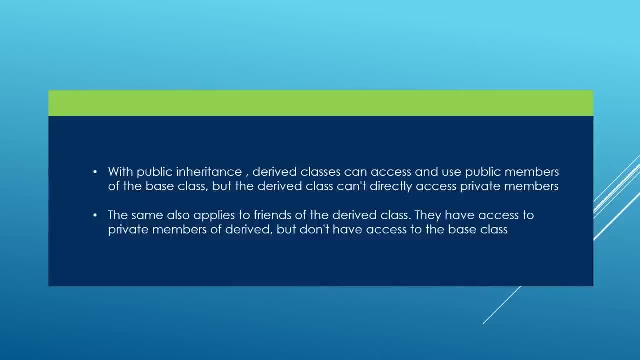 going to see what this gives us. so, with public inheritance, derived classes can access and use public members of the base class, but the derived class can't directly access private members from the base class. i want you to let this sink in what this means: from the player class we can't. 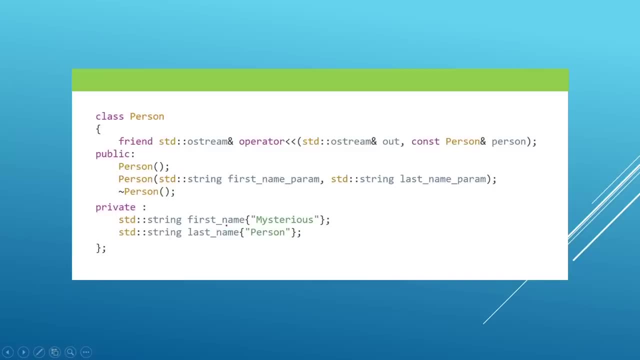 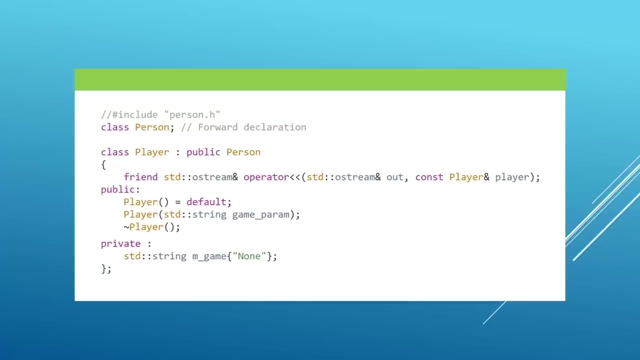 directly access the private member variables we had in person. remember our first name and last name are private to person and we can't directly access them in any deriving class. that is doing public inheritance. okay, so in our player class, if we try to access the first name and the last name, 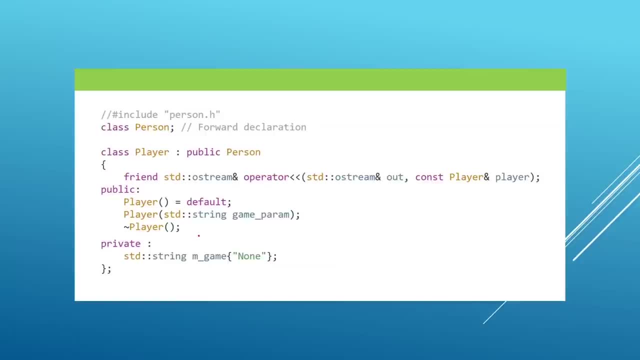 we're going to have compiler errors because we can't directly access them. but not to worry here we can still go through the public getters that we have in the person class to access the private member variables from the base class, and that's what we're going to do in this lecture here, because we don't have access to. 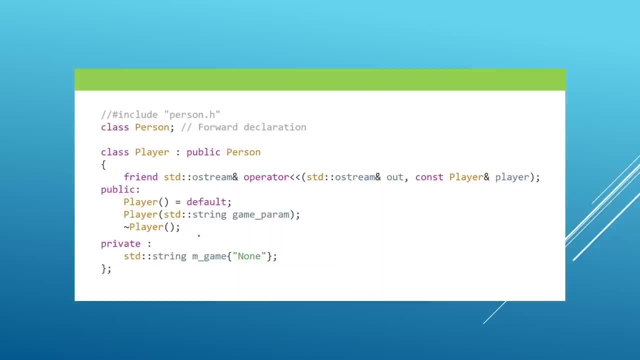 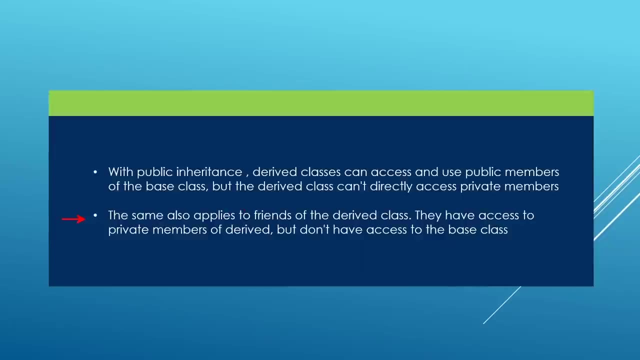 more powerful tools we're going to learn about in the next few lectures. the same is also going to apply to friends of the derived class. they are going to have access to private members of the derived class, but they don't have access to the private members of the base class. if you try to 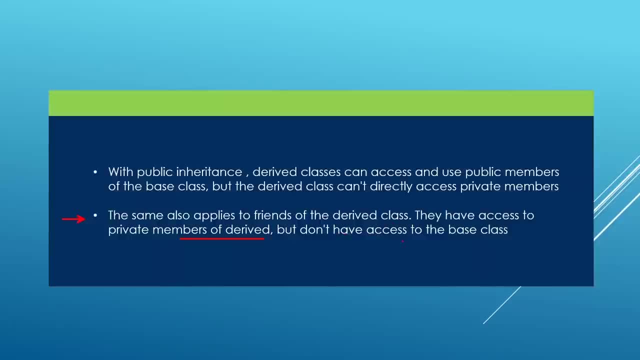 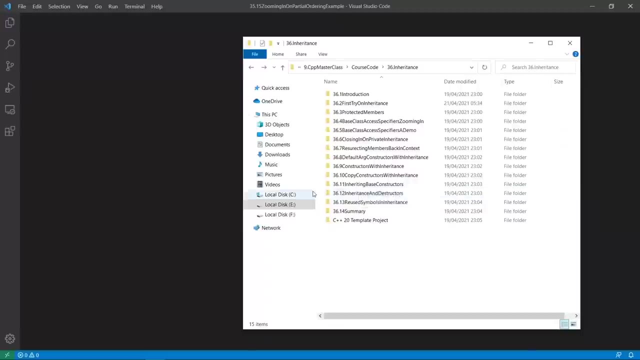 access the private parts of a base class from a friend of the derived class, you're going to have a bunch of compiler errors. okay, now that you know this, we're going to head over to visual studio code and play with this a little more and really drive this home. here we are in our working folder. the current project is first try on. 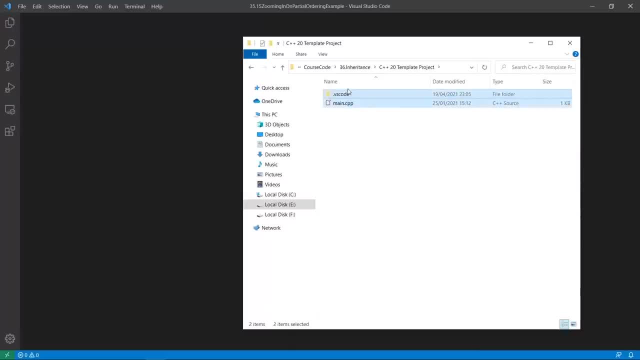 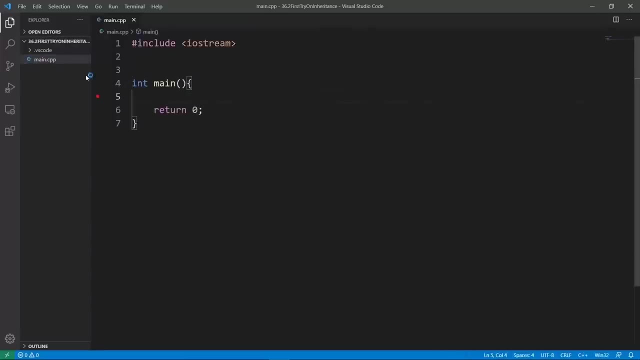 inheritance. we're going to grab our template files and put them in place. let's do this and we are going to open this in visual studio code pretty quick by dragging and dropping here and we're going to have our main cpp file. we can clean this up a little bit and we're going 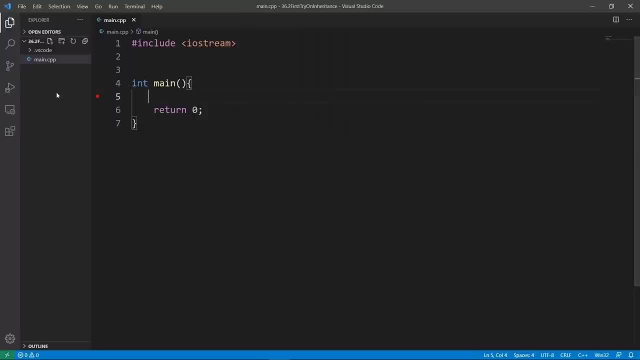 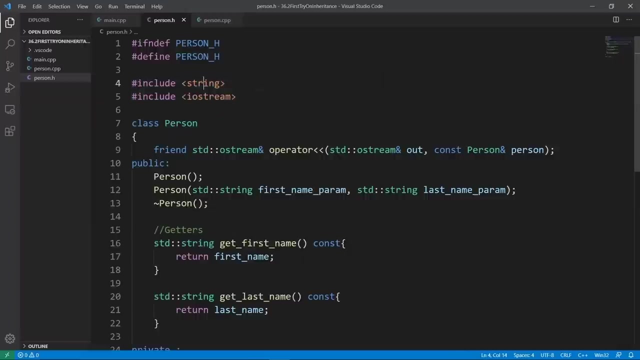 to add our classes. the first class we're going to add is the person class, so we are going to create its header file and let's do the cpp file. i am going to grab the code i have lying on my drive for the header. here i am going to put the class in. we are including the classes we're going. 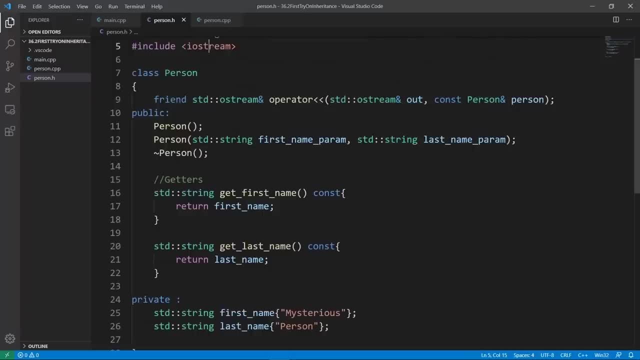 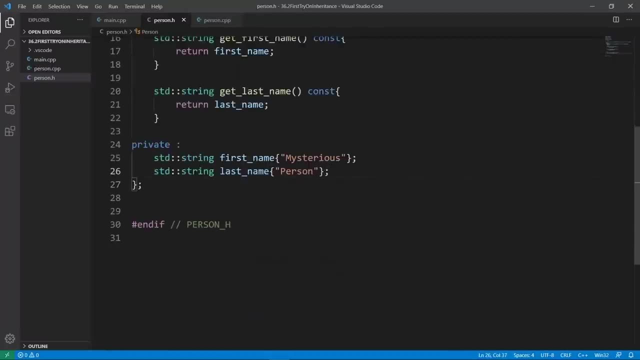 to need. we need string and i o stream here because we're going to be outputting thanks through the output stream operator and down here we have our two member variables. we have first name and last name. they are of std string type and we have a bunch of constructors here. 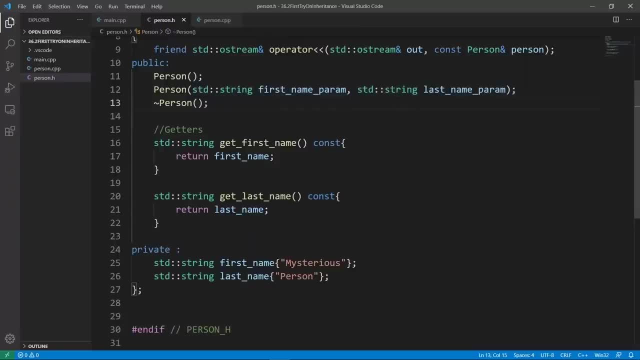 a default constructor and one that takes two parameters. we are taking them by copy here. this is bad. we should at least pass them by reference here. let's correct this pretty fast, and we're going to make the second one a reference as well. let's do this. 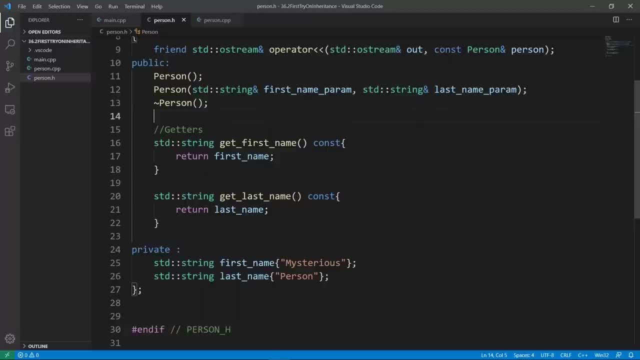 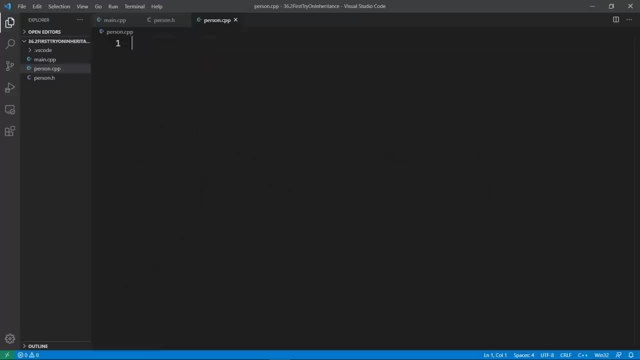 and we have a destructor which is going to do nothing because we really aren't doing any dynamic memory allocation here. we're going to head over to the cpp file and put in the code for that. we're going to include the person and we're going to do our constructors put in the implementations. 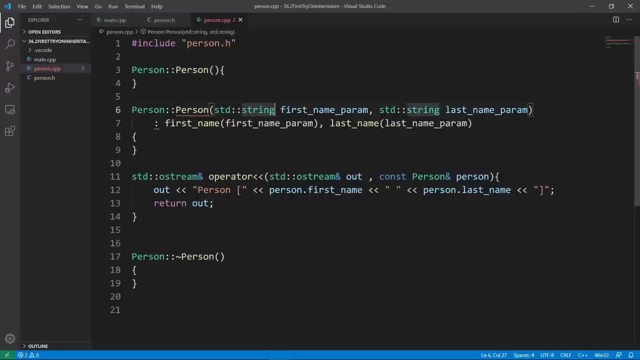 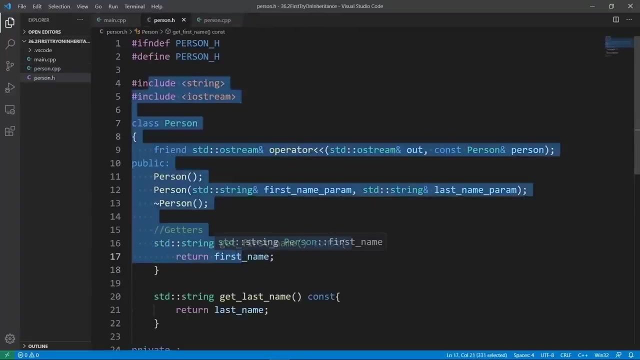 i should say- and we're going to pass our parameters by reference again, let's do this, and our constructor should be done. now we have a personal class that we can use to derive other classes and use this class as a foundation to build other classes. to visualize this again, our 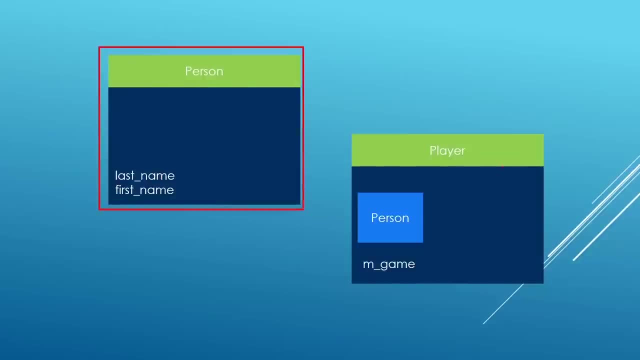 class person is going to be the base class for our player class. so if we build a player class, it's going to have a person part of it which is going to be the foundation on top of which we're going to weld. notice that in player we don't need to set up last name and first name. they are going to come. 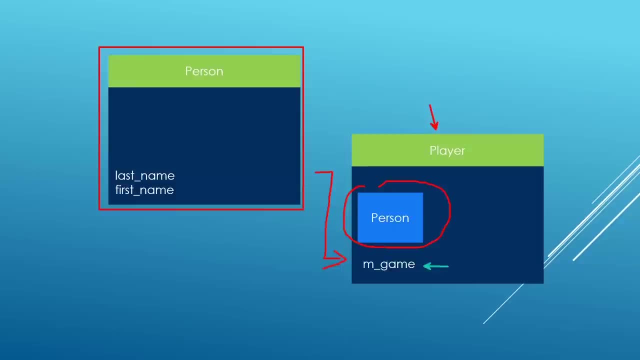 in as a player. all we need to do in player is set up the game member variable to make him a full player who can have the game they happen to be playing. this is the idea here. okay, so now that we know this, we're going to put in our player class. we're going to create the files for it. 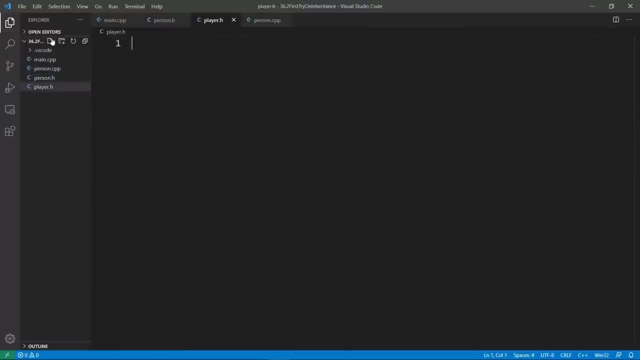 let's do player dot h. we're going to put this in. and we're going to do player that cpp. we're going to put him in. we are going to hop over to the header file and put in our code. the class is going to be player and it is going to be inheriting from person. this is the. 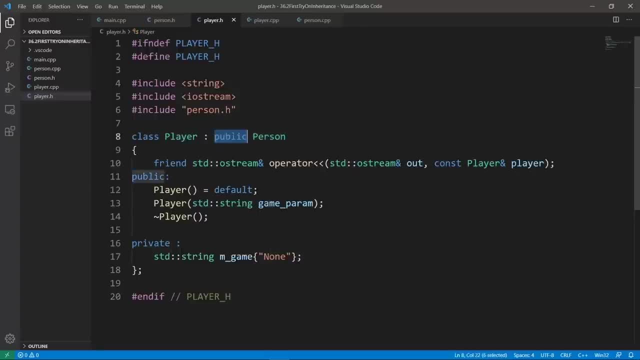 syntax again. we say colon, colon. we say the kind of inheritance we want to do- in this case it is public- and then we say the class that we are going to be inheriting from, from this point on, the player class is going to have a person part of it, and we are going to prove this in a minute when we 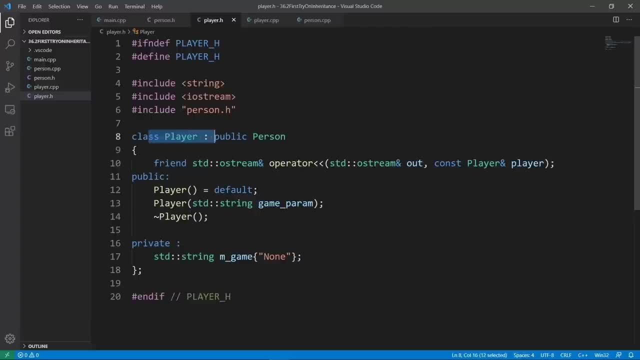 run this code here, notice that we can build the player objects by just passing in the game a parameter here which is going to be used to initialize our member variable. let's also make it a reference because this is good practice. it is going to avoid copies. you can even use string. 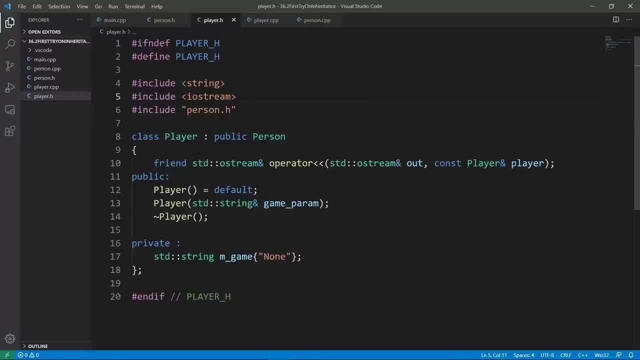 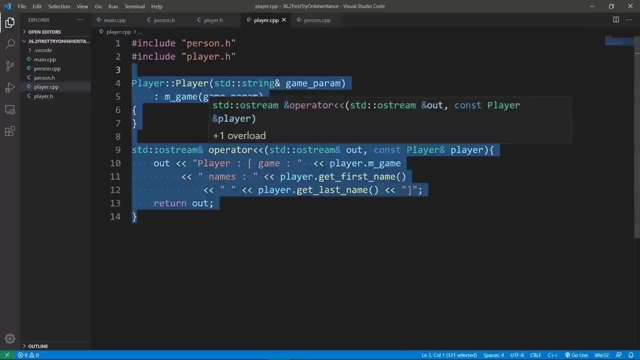 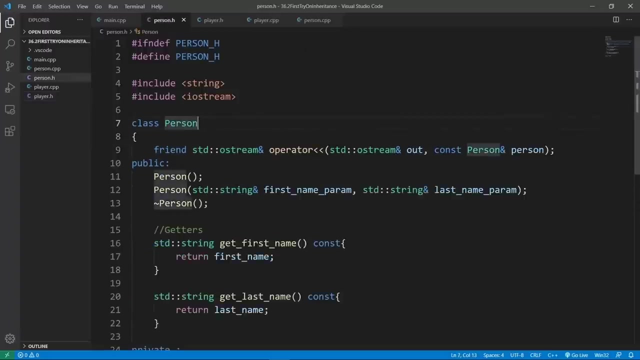 views, but that's going to be your choice. we are going to hop over to the cpp file and put in our implementation and this is going to complete our setup for the player class, which is going to be inheriting from our person class. here we can actually head over. 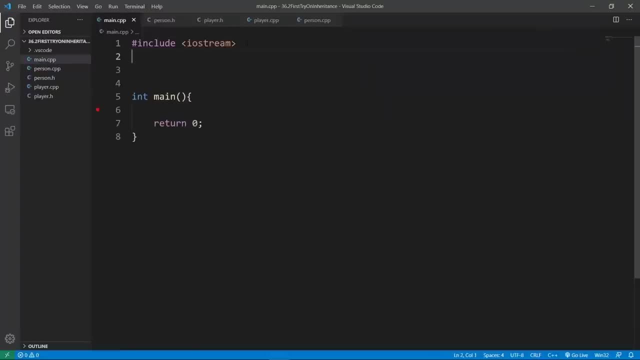 to the main cpp file and include the player class. let's do this. we're going to say player and we can create player objects. let's look at the code again. for a player, we have a constructor which is going to take a string parameter. we can use this to create a player and specify the game. 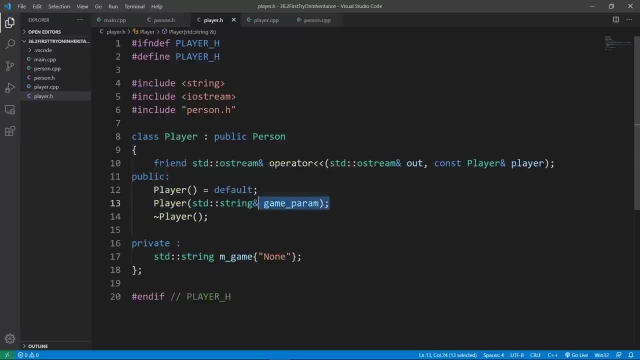 they are going to be playing, but for now we don't have enough tools to put in the data that would initialize the member variables in the base, the class, which is person. here, if we go back to person, we're going to see that we have the first. 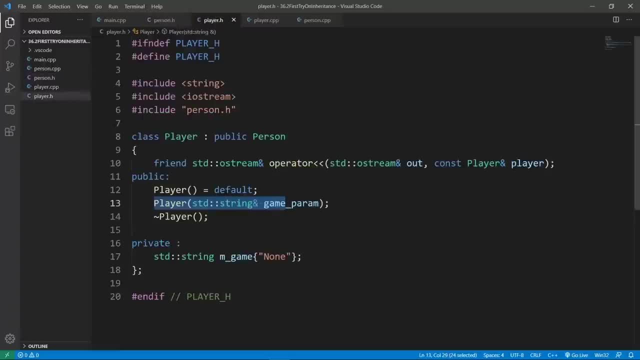 name and the last name. but in our player class these member variables are going to be inherited because a player is inheriting from a person. this is the syntax to do that. but even if the player class has a person part inside of it, we can't really access private members from person from. 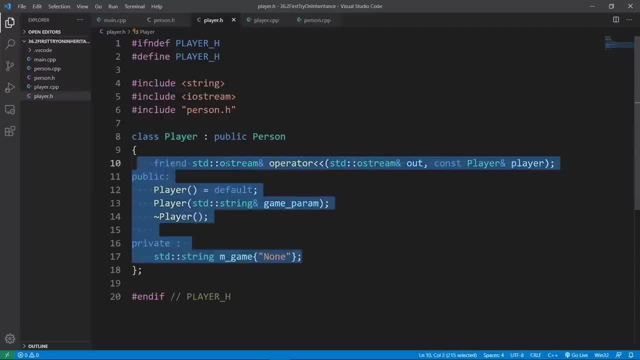 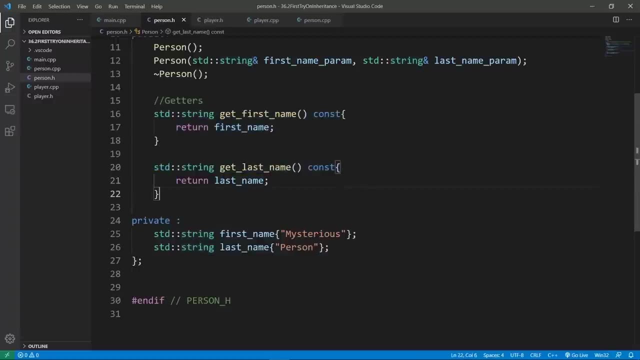 a player object. we're going to see a few ways we can get around this, and one of those is to go public methods from the person class to access private parts of the person class. this is going to give us access to these member variables. if you go down in our stream output operator, you're going to see that we are using. 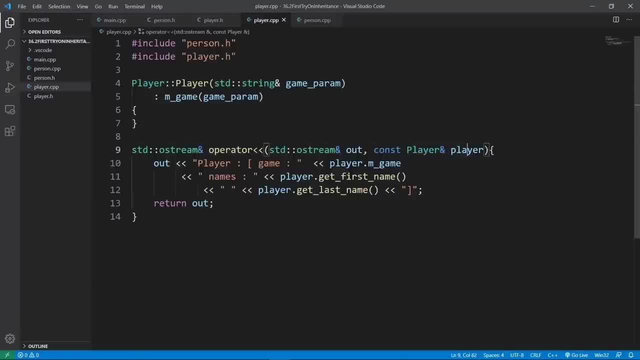 these getters here. the parameter is a player objects that we want to print out, but to get access to the names, we are getting the first name and the last name through our getters here. before we really explore this any further, i think it is a good idea to go in. 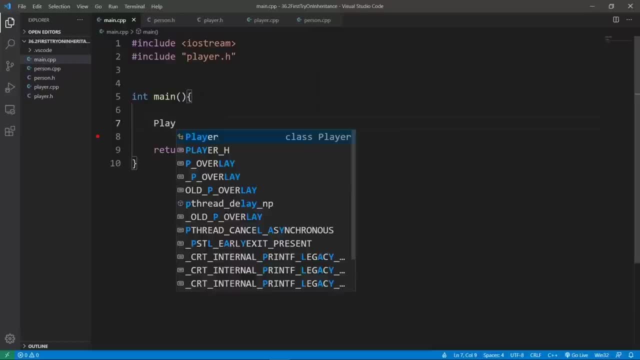 the main cpp file and create a player object. so we're going to do that, we're going to say p1 and we're going to specify that they play basketball- why not? okay, so we have our player object and we can really do all we want with it. for example, we can print the information about this player object. 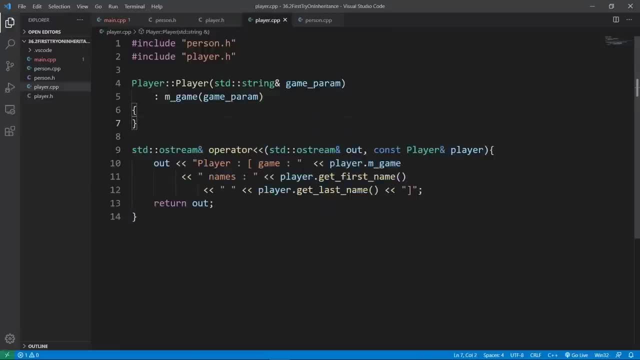 if you remember, in player we have a string output operator which is going to print all the information, and here we have a problem because this guy is taking the data by reference and this is not the reference. this is a temporary object that we are passing here, so we could go back and change this to take a string view parameter. 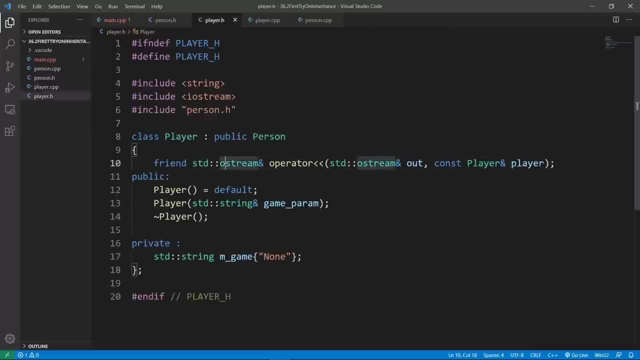 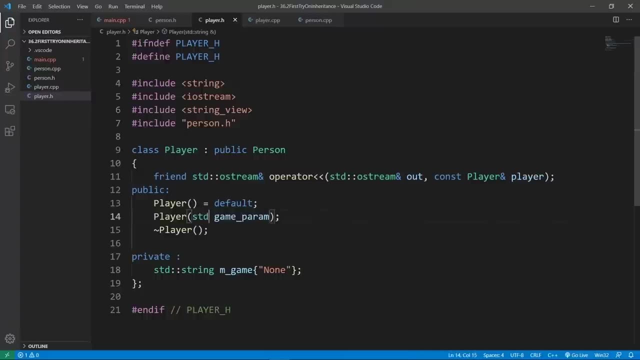 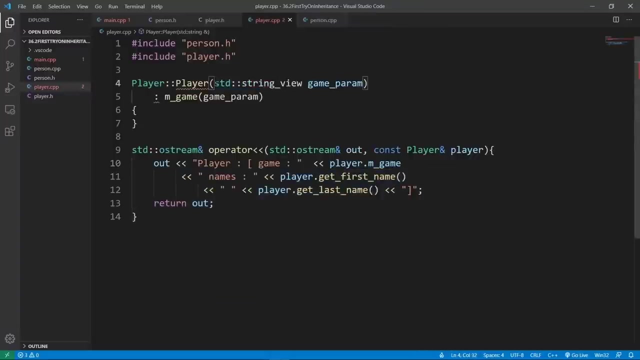 let's go back and do that. we're going to include a string view here in player and we're going to change our parameter to be std string view by value and we're going to do that in the cpp file. let's do that. we're going to say std string view and this should take care of our problem here you. 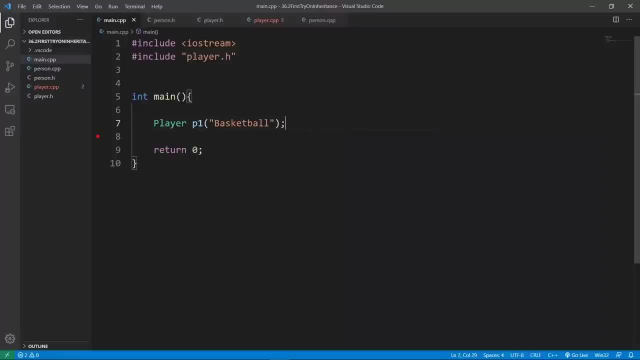 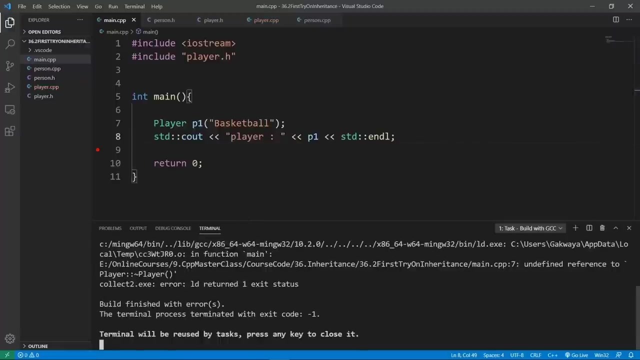 see that the problem goes away. now that we have this guy, we can print it out, we can say stdc out player and put the information out. okay, so now that we have this, we can try and build our program. we're going to use gcc- you our favorite compiler- and you're going to see that we have a problem and defined reference to. 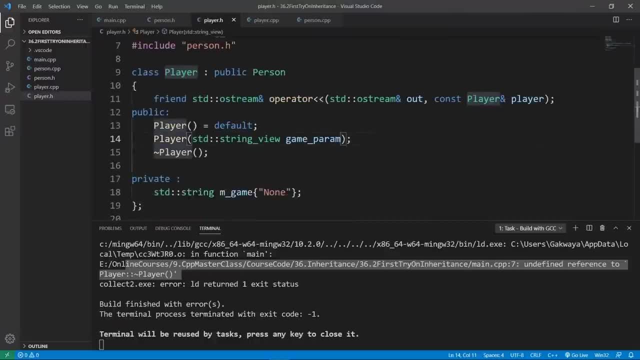 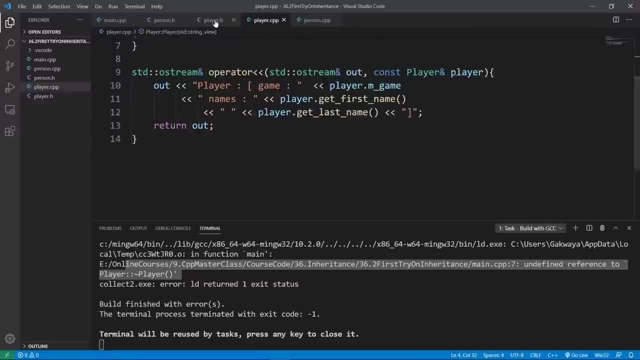 player destructor. let's go back in the hair and see that we have a destructor, but we probably didn't put a destructor in the cpp file, so let's do that. or because we're not doing any dynamic memory allocation, we can even completely take out this destructor and we're just going to use the. 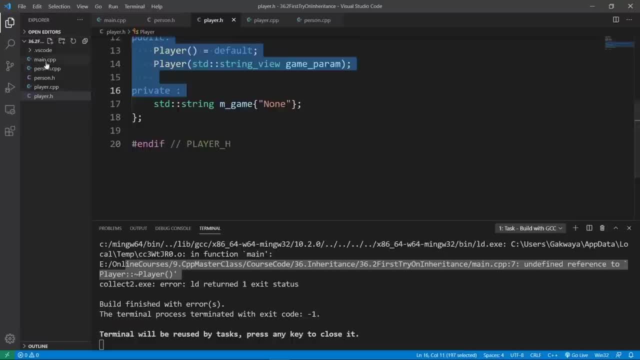 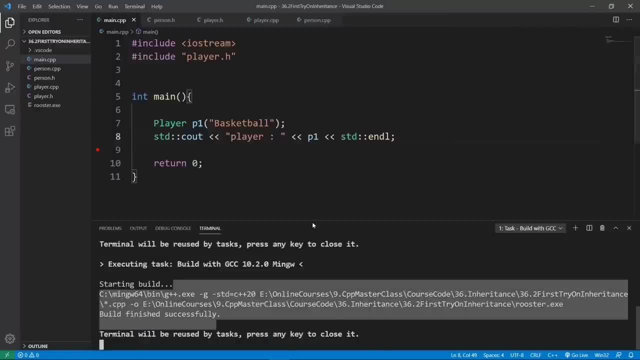 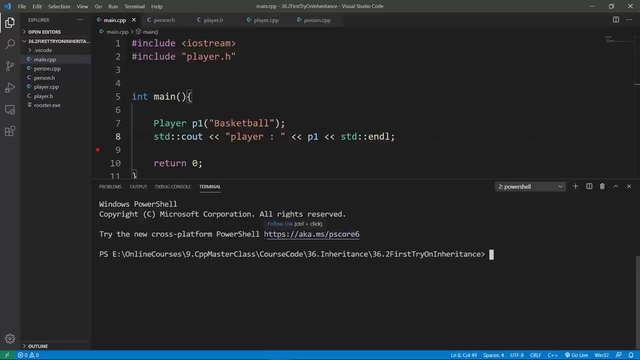 one the compiler generates for us. this is going to be much easier to do, so let's go back and see what we can do in our code so we can build again with gcc. okay, the world is good. we can run this program. and let's see if we have a powershell window. we don't. we're going to bring up a new one. 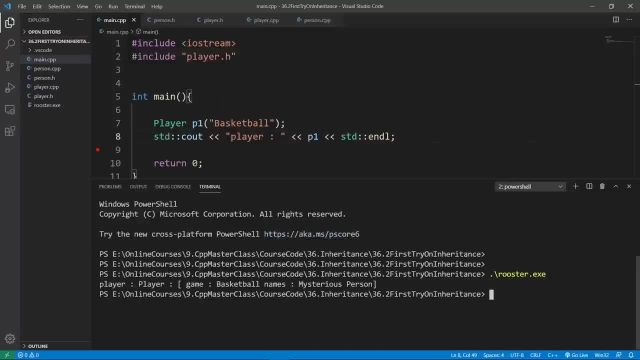 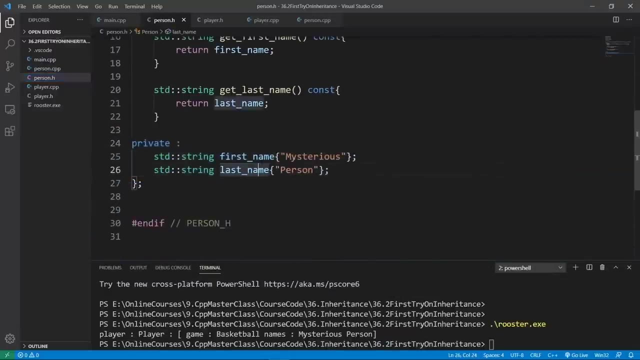 and we're going to run rooster, we should see information about our player. so, player, the game is basketball. the names are mysterious: person because that's the default data we inherit from a person. if you go back to person, you're going to see that the default data in first name is mysterious. the default data in last name is person and it is what 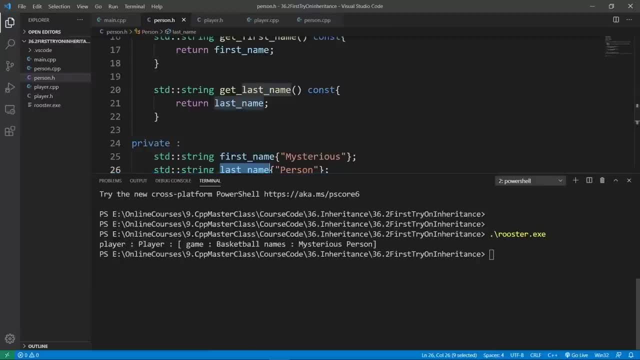 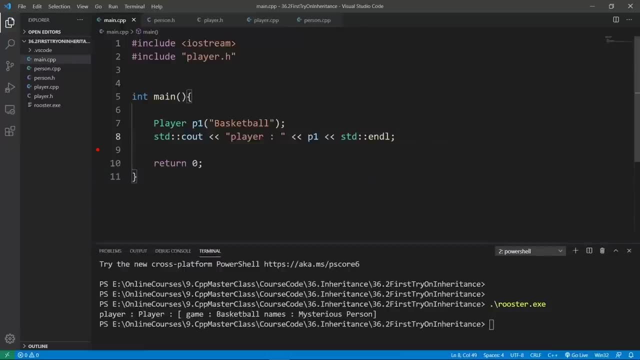 we see printed out here in our powershell window when we print information about our player object. another thing i want you to see is that we can actually really prove that any player object is going to have a person part of it baked in and that's going to be storing the. 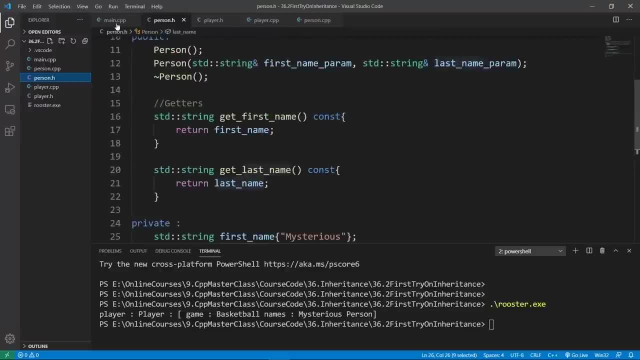 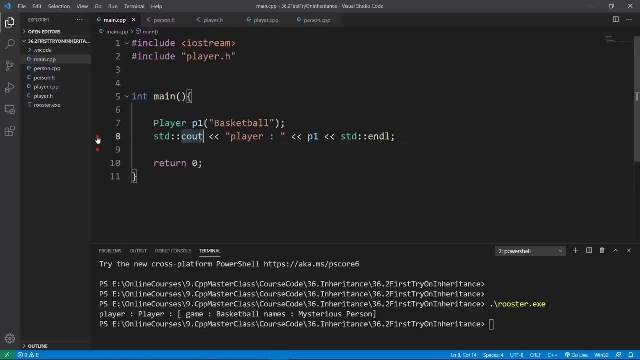 information that is modeled into our person class and we can use a debugger to do that. for this to work, i am going to put a break point here, on line 8, which is printing things out. this break point is going to be hit after our object is set up and we can really see the data. 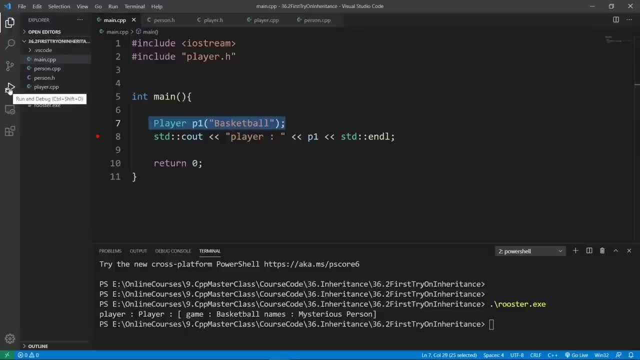 inside this guy here. so what we're going to do, we're going to hit this run tab and we're going to use g plus plus. we're going to use the debugging tools here and we're going to use the tools that come with gcc, because this is our favorite. we're going to hit the green button here. 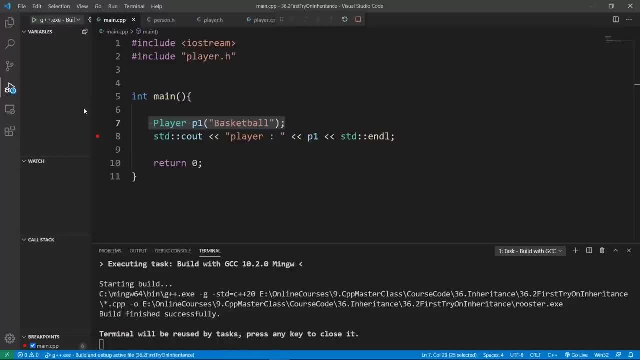 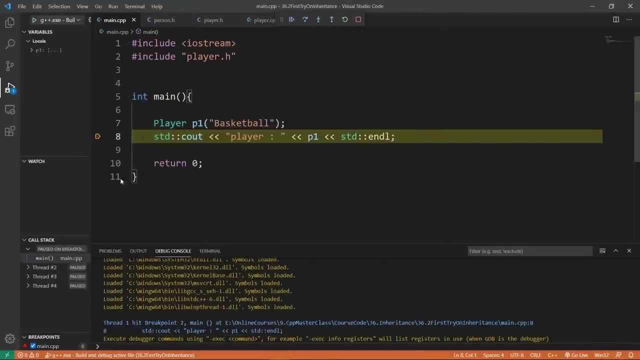 this is going to start our debugging session. a binary is going to be built and it is going to be plugged into our debugger, and we're going to hit our break point here now, if you look on the left here, you're going to see a title that says locals. we're going to expand this and we're going 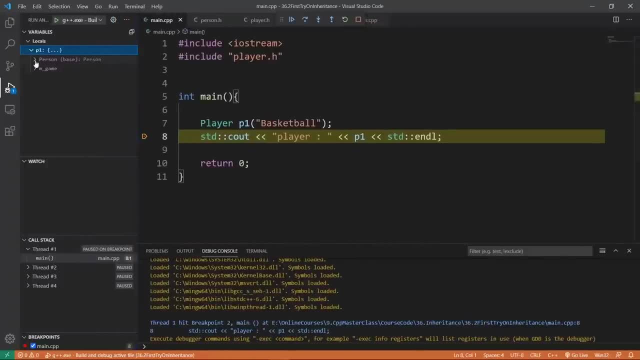 to see that the p1 object actually has a person part of it. and you see that visual studio code is being held up here and we're going to hit that, and we're going to hit that and we're going to see that we have our member variables. we have first name and last name and this is a player. 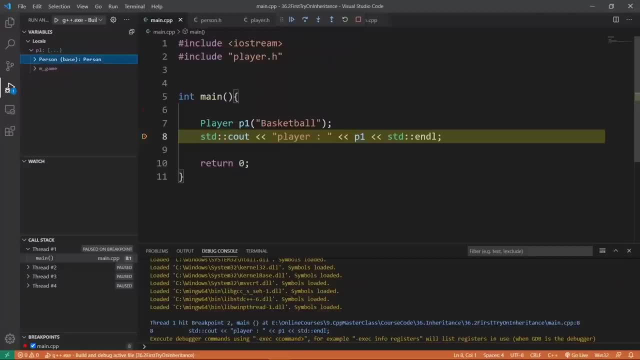 object that we are looking at. don't forget that. and on top of our person part, we also have our own member variable, which is the game that we play, and it is right here. hopefully, this proves to you that any derived class object is going to have a base part embedded into it, and we're going to 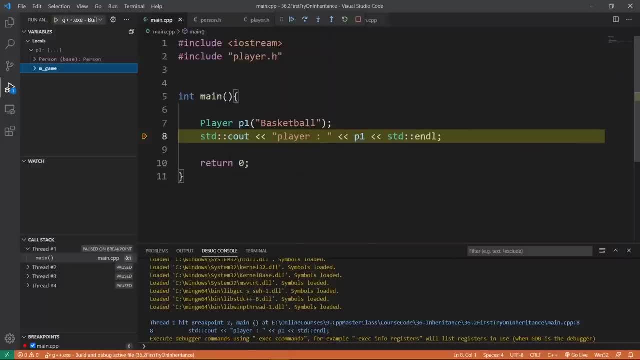 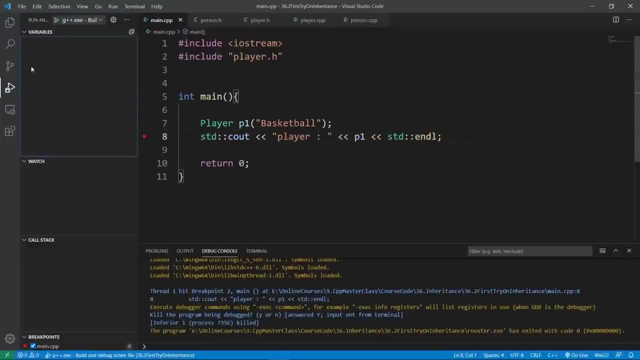 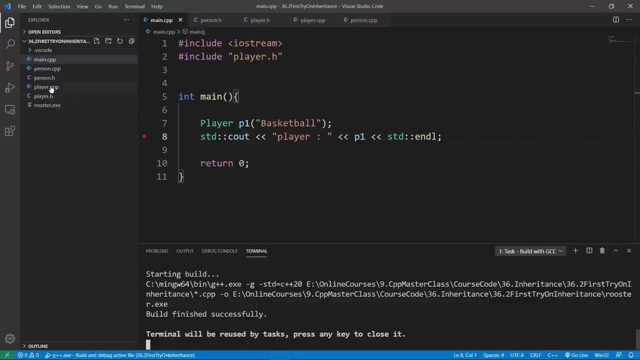 hit, and that's going to be the foundation on top of which the derived class is going to be building its own thing. this is the basic idea here. okay, now that you've seen this, we're going to kill our debug session and we're going to see some of the things you need to be careful about when doing. 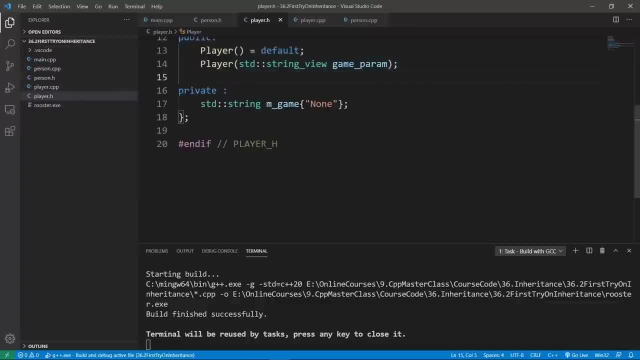 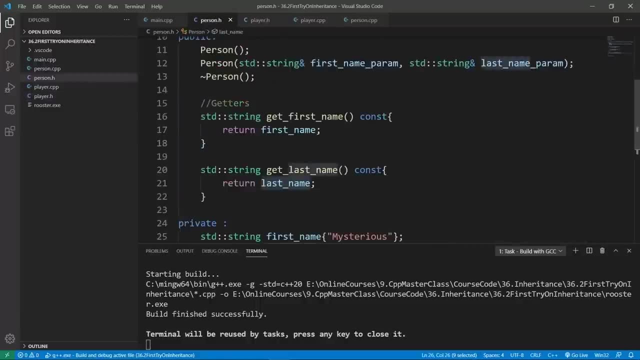 public inheritance, like we are doing here. the first thing i want you to see is that you don't have access to private parts of the base class. if you go back to person here, let's kill this so that you're not confused. if we go back to our personal class, we're going to see 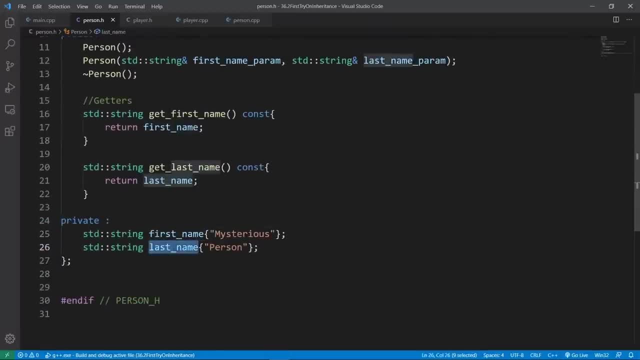 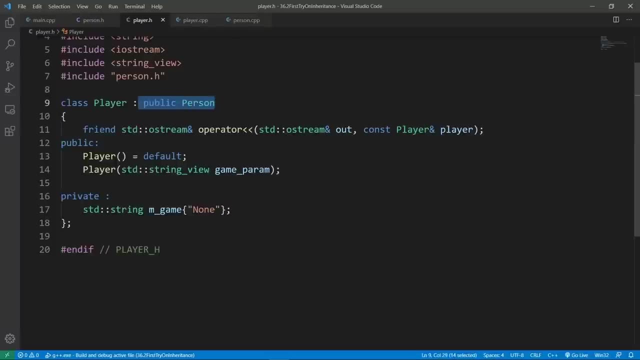 that our first name and last name are private, so they want to be accessible to any class that does public inheritance, like we are doing here. they are just going to be private. they are going to be part of the class, but the derived class would have access to them. this is the idea. 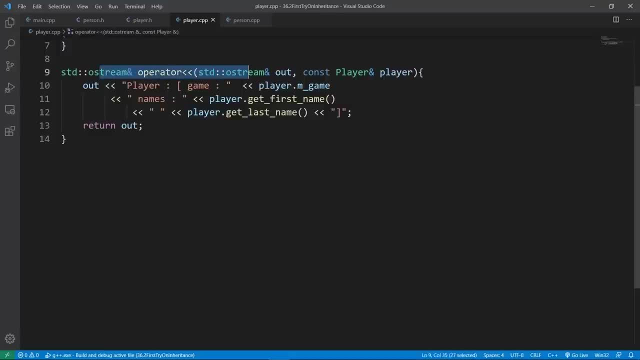 here and if we go in our output class, we're going to see that the derived class is going to be private and we are going to see that we are going to have access to our single and only class. now let's look at another example. let's go back and look at this code: trim, operator and comment. 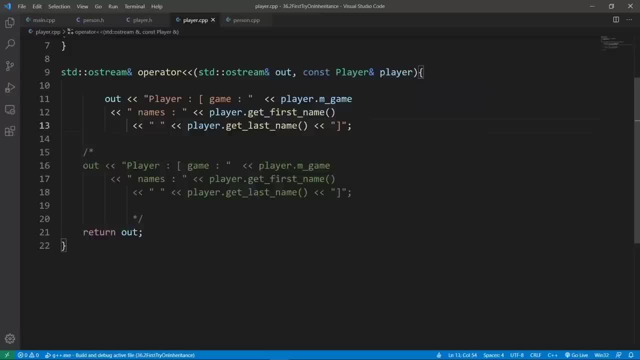 out what we have here and try to directly access these member variables. let's do that. i am going to copy the code here and put that on top and we are not going to go through the gateway methods from the base class. we are going to try and access mfirstname. let's go back and look at. 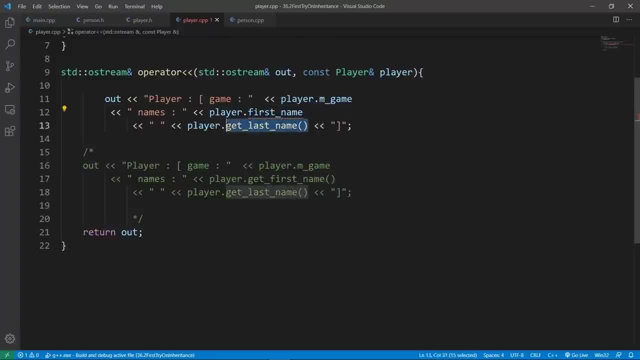 the names for the member variables. it is firstname and last name. let's use that. we're going to say first name, see that through user name here. and we are going to copy this to third class and see what intellisense but trying to access that is going to give us squiggly lines. you see that we have this. 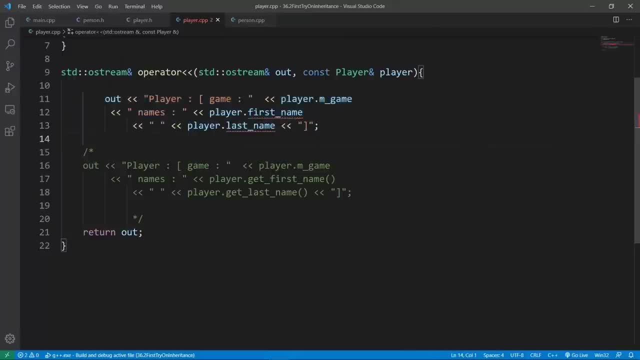 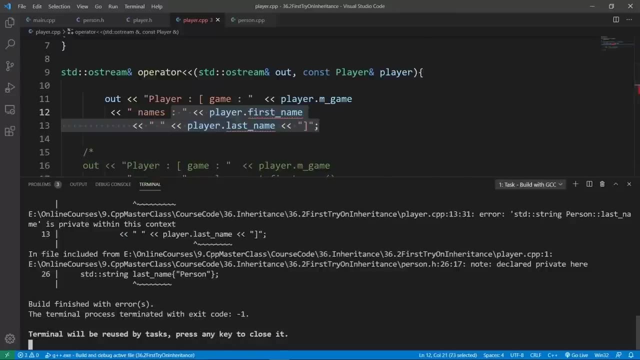 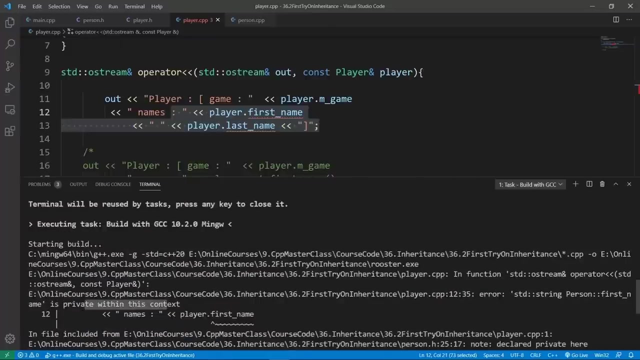 in our autocomplete but we have squiggly lines. we can't access these. if we try to compile our program, let's do that again. we're going to use gcc and we are going to get compiler errors and the compiler errors are basically going to say first name is private within this context again, 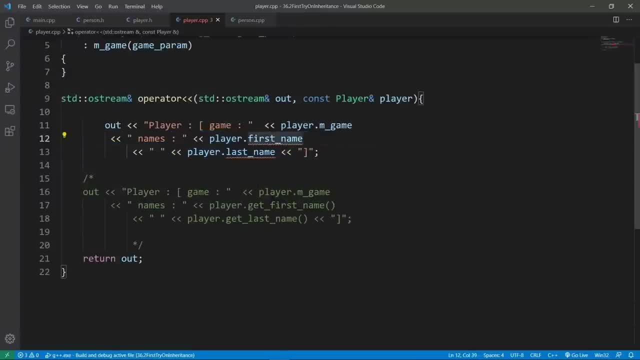 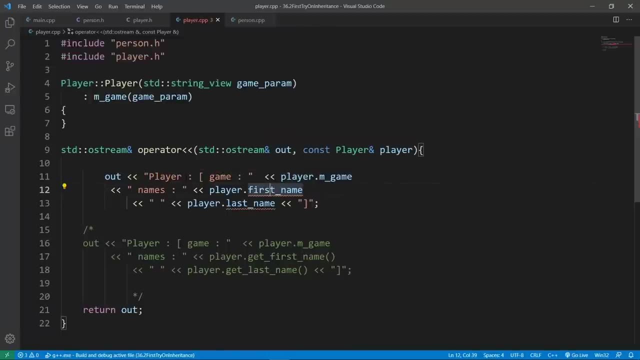 the meaning is that first name is private to the base class and we have no business accessing that in a derived class, which is the player class here. this is the meaning, so we can't really access that. okay, i realize this is a global function, but even if we try to do that from 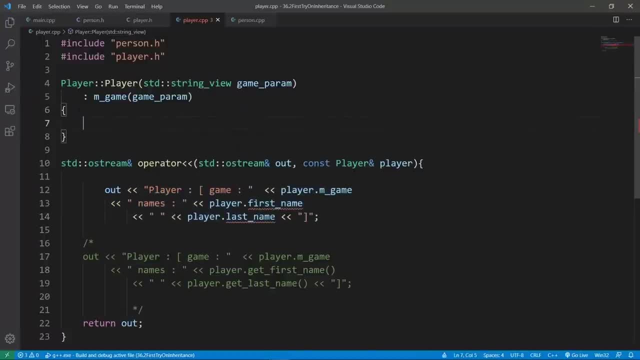 a member function, let's do that from a constructor. we're going to try and say first name. okay, i realize the access we are trying to do from the output stream operator is really not a good example, because this is not a member function, it is a global freestanding function, so we can try and change the first name and last name from. 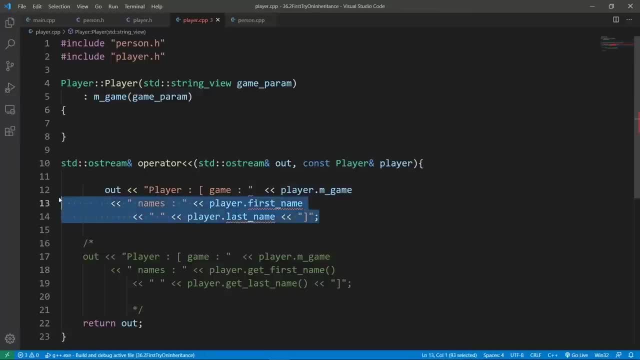 the constructor, for example, and we're going to see that this is not going to work either. so we can take this out and we're going to remove our block comment. so we're going to take out what we just did here and we're going to uncomment our good code here, which is using getter member. 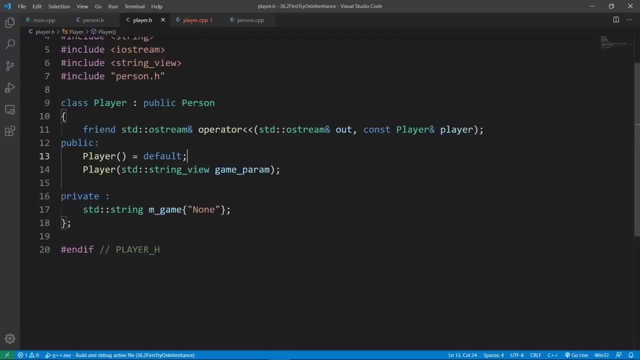 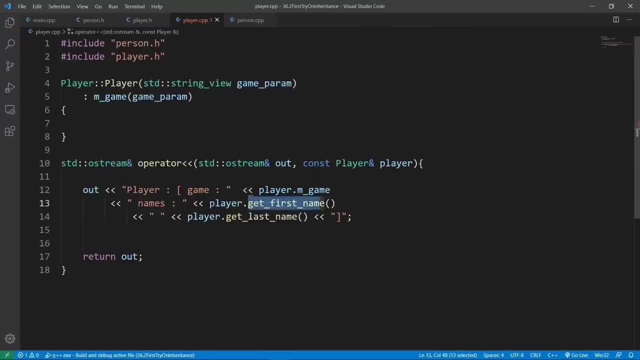 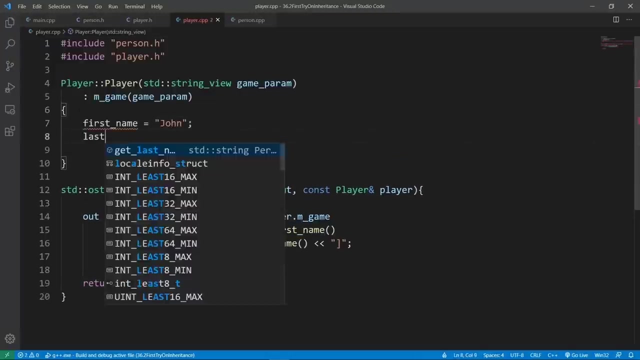 functions from the base class and we're going to try and change the first name and last name from the base class and change those into our constructor of the derived class. we're going to try and change, for example, the first name and make it john, and we're going to take the last name and change that. 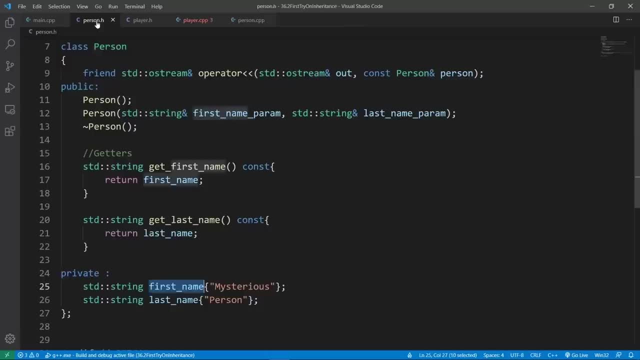 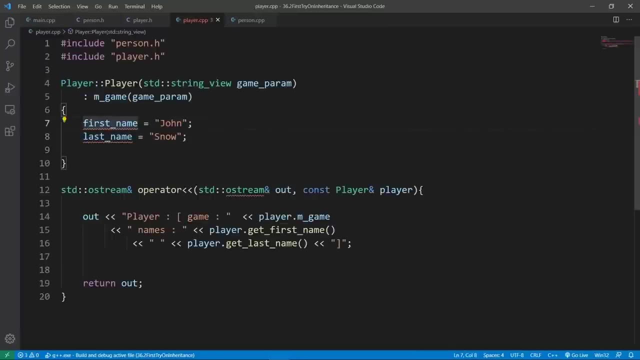 to snow. let's do that and let's go back and make sure we have the correct names and you see that we have squiggly lines. we can't really do this because these are private members of the base class and we can't access them from a derived class. they are part of the player class. 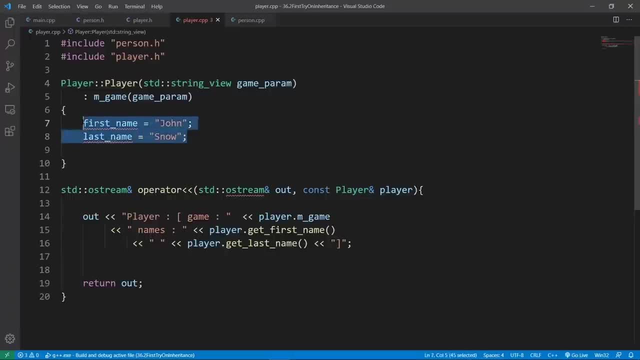 which is a derived class, but we don't have access to them. we can't modify them or do anything. we can't read from them, we can't write from them. this is the message here. if we try to build our program, we're going to use gcc to do that. we are going to get compiler errors and let's see. 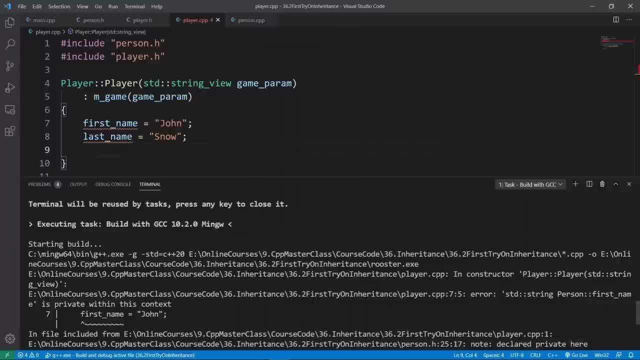 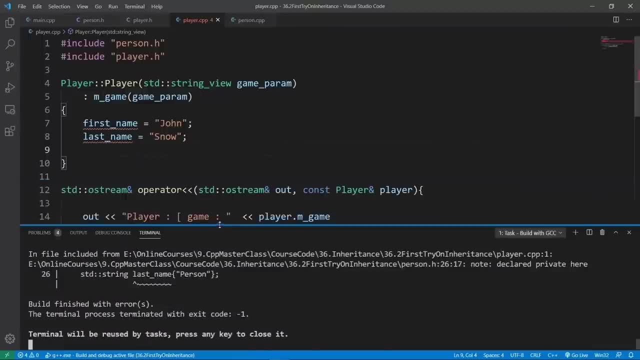 the compiler error, we get again. the error is that first name and last name and we're going to get our private to the base class and we have no business accessing them from a derived class like we have here. so if you need any kind of access to a private member of the base class, 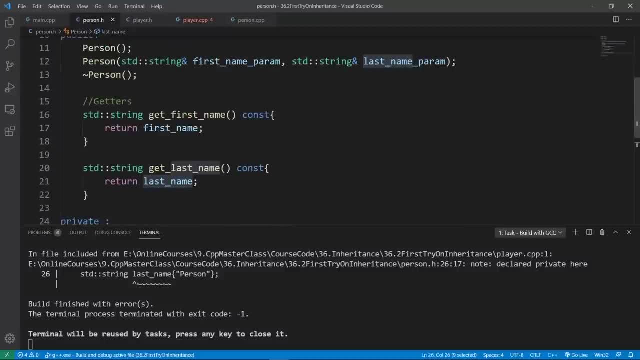 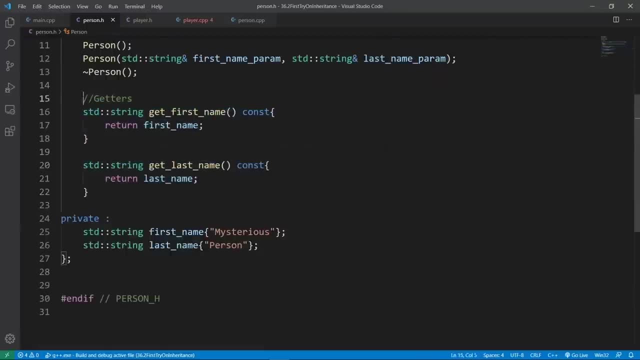 you will have to go through something that is public, and a good example is getter methods, which are going to allow you to change things. so, for example, if we want the ability to change the first name and the last name, we can set up a bunch of setter methods. let's do that. we're going to 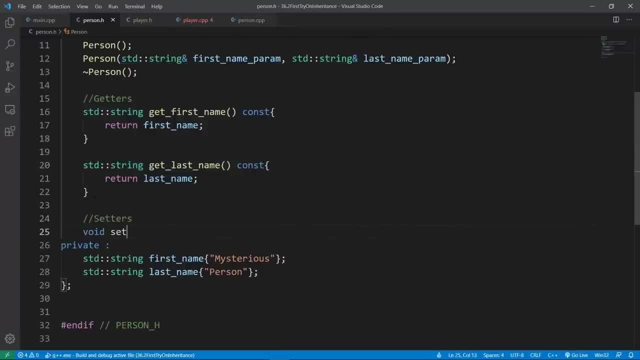 say setters and we're going to say void set first name and we are going to pass an std string view. let's do that. we're going to say string view here: fn for first name. this is going to modify our class, so we are not going to mark this as a constant member function and we're going to say: 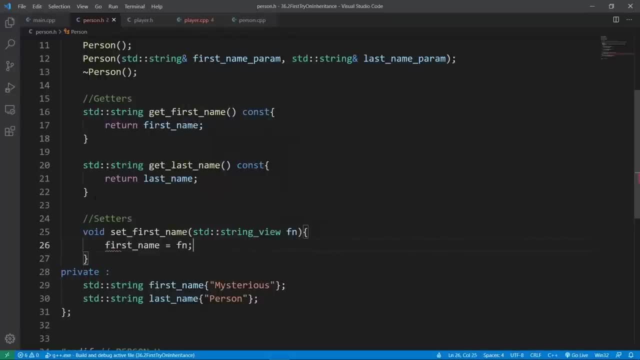 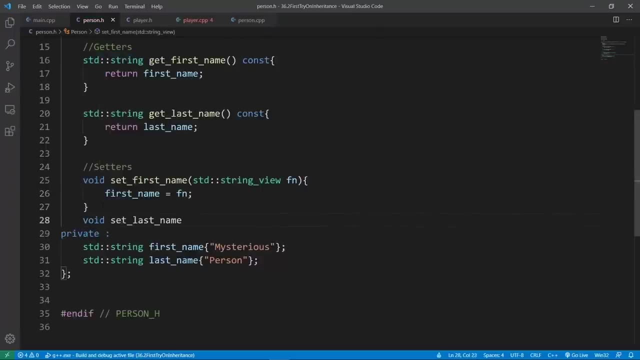 first name equals fn. this is going to do. we are going to set up a setter for the last name set and we're going to pass a string view here and we're going to say ln for the last name. again, this is not going to be a constant member function, so we're going to say: 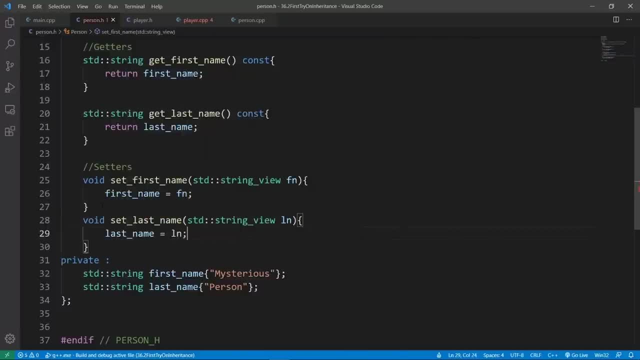 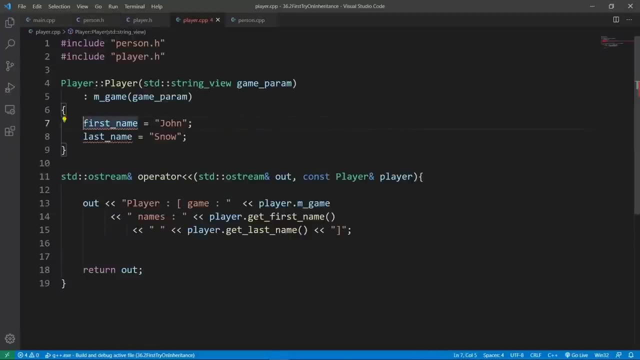 last name and we can pass in ln as our new name here. now that we have these in, we can take out these things we have in the constructor. i think the job for this is done and this is going to give you compiler errors and we can go in our main cpp. 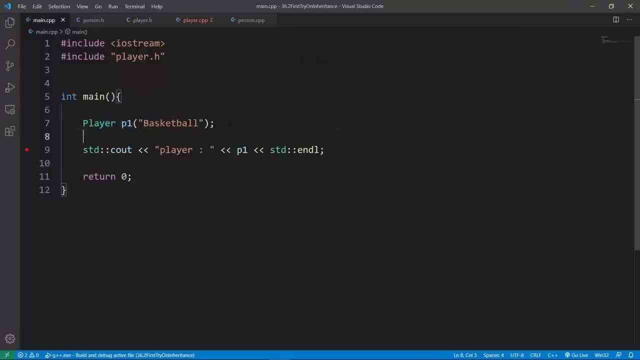 file and change the names for this person. here, for example, we can say p1, set first name, we're going to pass john and we can also set the last name. we're going to say p1, set last name and we're going to pass snow and this is going to do. if we build and run this program, we're going to see that 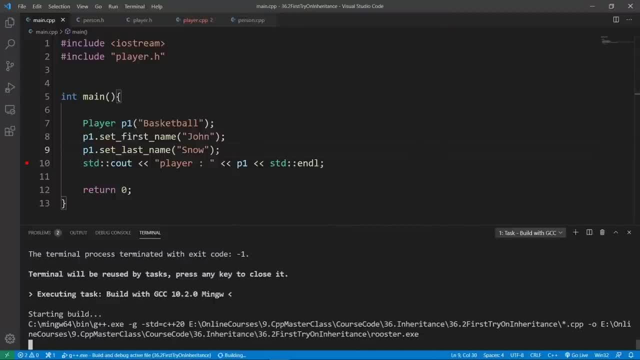 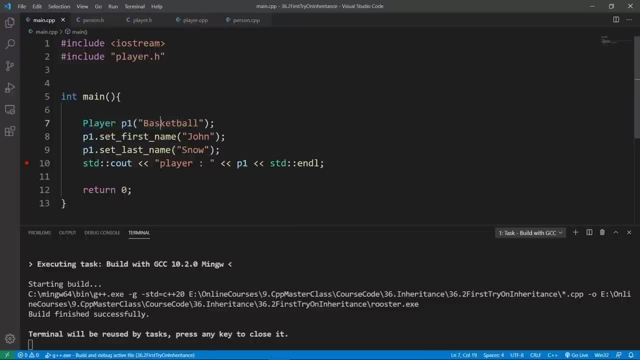 the build is going to be good. this is the first step and if we run, we should see the information printed out. we want to join snow printed out. the game should be basketball. let's clear and run rooster. we're going to see that the data is in here. 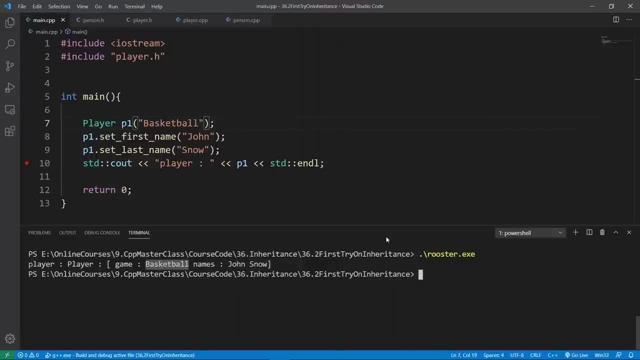 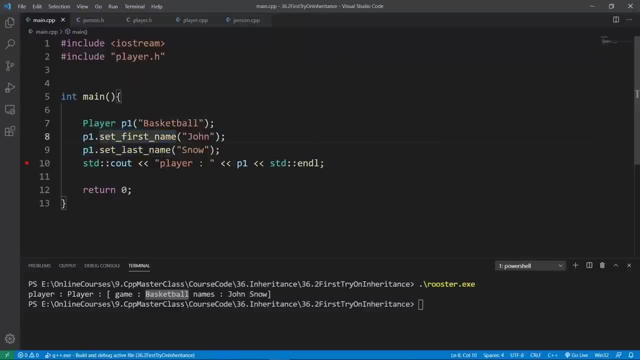 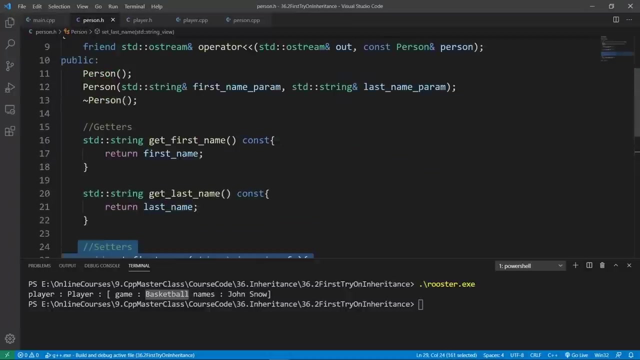 the name. the names are john snow and we have our game to be basketball here. but notice, these are base methods and we are calling them from a derived object and this is living proof that the public members from the base class are going to be inherited and usable from a derived class. 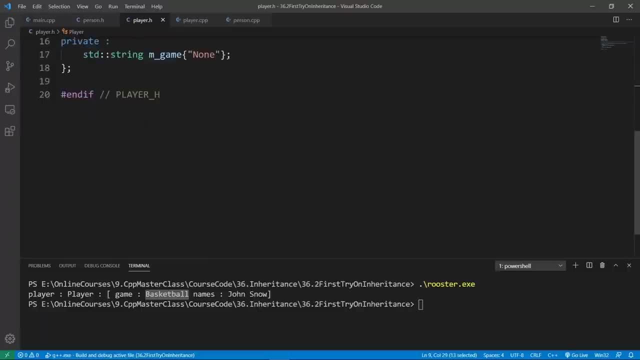 that does public inheritance like we are doing here, and this is really the main message. you can inherit publicly and have access to public stuff from the base class and use them in your derived class, but private data is going to still be private to the base class. you can't use that in a derived. 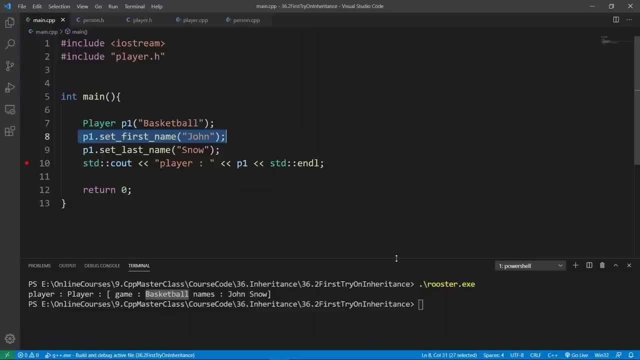 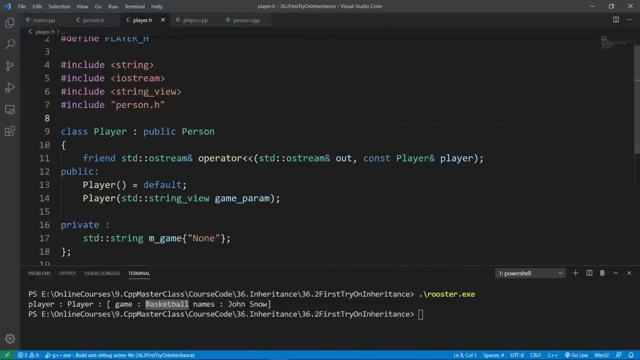 class. this is the message here and this is really all i wanted you to see in this lecture. the big thing is to notice the syntax you use to do inheritance, and if you do everything in this lecture, you can do everything in your derived class. so, basically, i'm going to 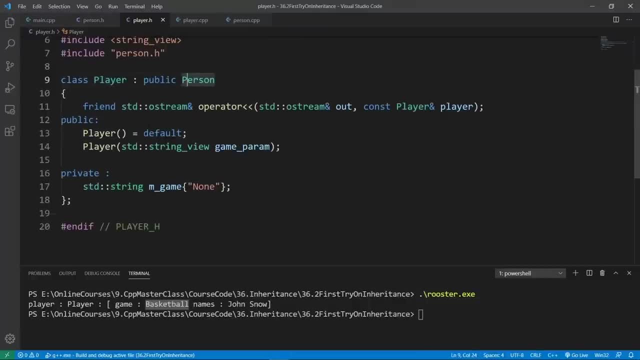 show you a little bit of how to do it with the basic class, because it's a very complex and very complicated thing. we can build together based on a database concept or based on a database concept. so let's build this database concept. like you see, we can build a database and we can add the link and we have the other. 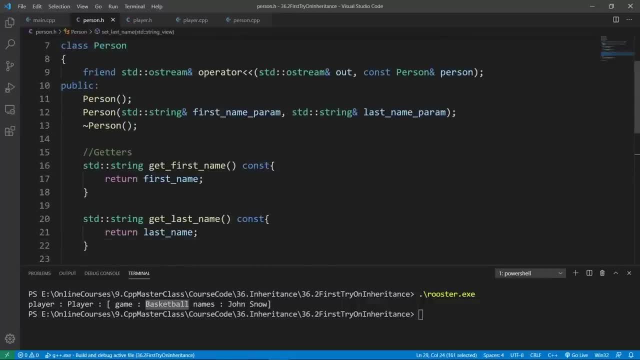 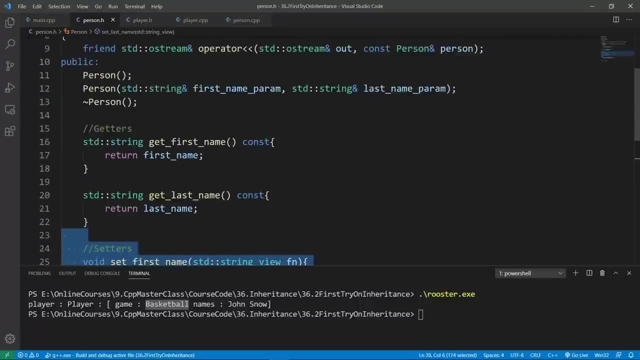 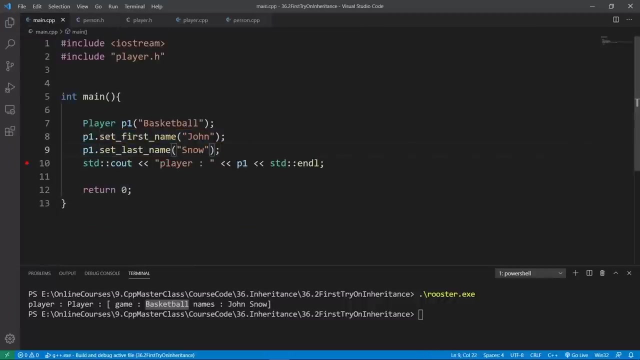 version of the database and we can create a Blazor code, we can create the range of variables, we can create columns, we can create all kinds of different kinds of variables. for that example, we can do the process and we can build the from the outside, because they will be inherited as public in a derived class. 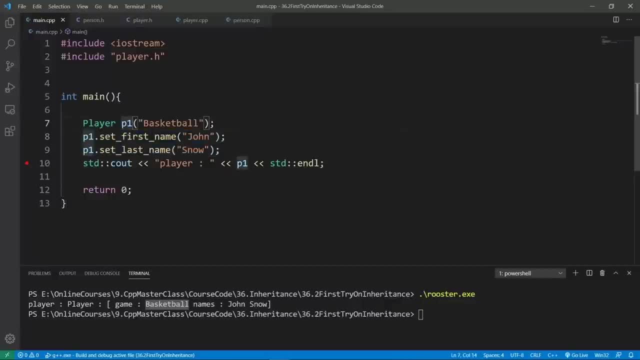 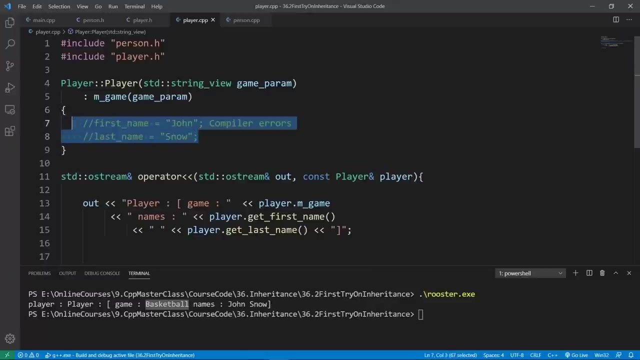 so we can really call these methods and use them from the outside, like we are doing here. but private data from the base class is not going to be accessible and usable from a derived class, and we saw that by setting up this piece of code in the constructor of player. this is going to give us a compiler error. 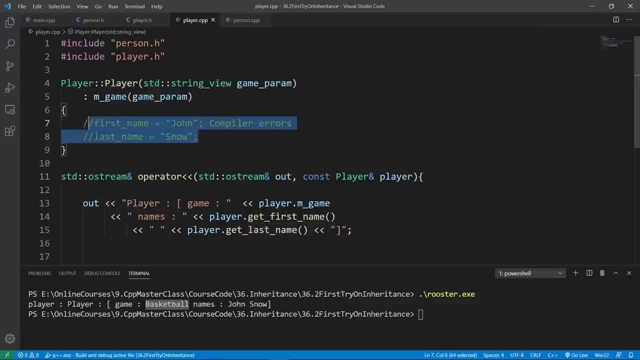 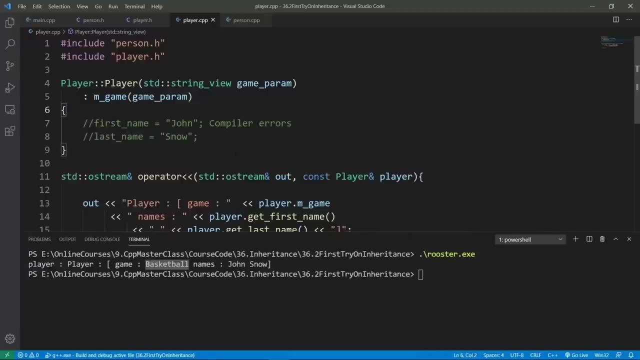 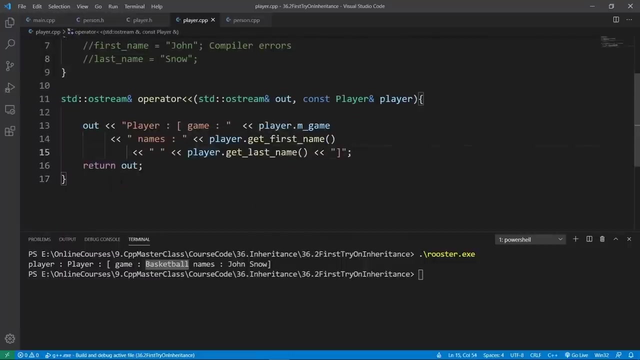 saying that first name and last name are private to the base class. we are going to stop here in this lecture. in the next one we're going to learn about another kind of access specifier we have in C++ and that is protected. so go ahead and finish up here and meet me there. in this lecture we're going to learn about the. 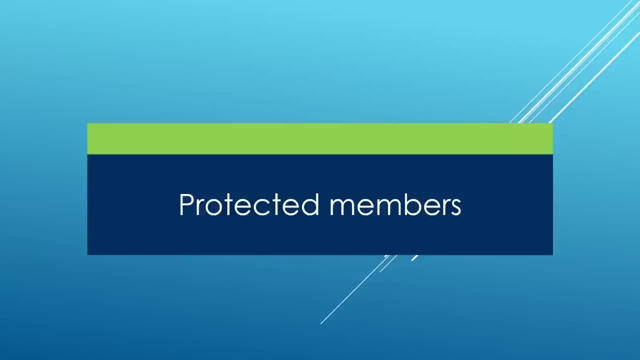 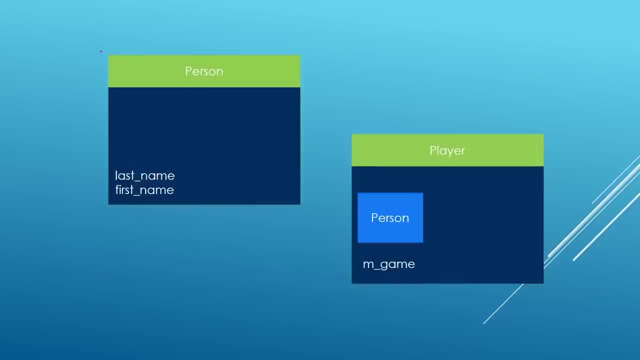 protected access specifier you can use in your C++ class and we're going to be reusing the same code that we used in the previous class and we're going to send out- and this is the setup we used in the last lecture. we set up a person class. 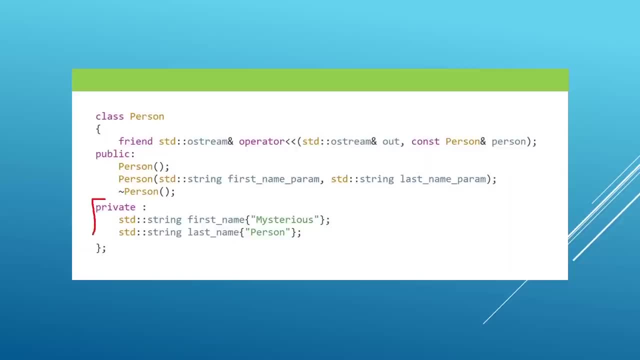 our members were private, as you saw here, but in the last lecture we saw that private member variables are not going to be accessible and usable from derived classes that do public inheritance, and sometimes we want members from the base class to at least be accessible and usable from a derived class but still be inaccessible from the outside, and we can achieve this using 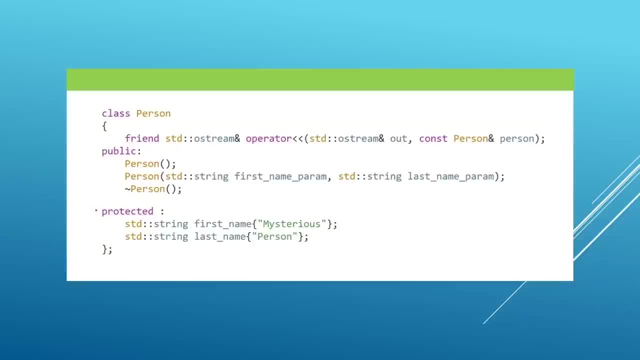 the protected access specifier. so, for example, we can change the access specifier of our member variables from private to protect it, and at the moment we do this, we will be able to access, for example, read from and write into these member variables from derived classes. so, for example, 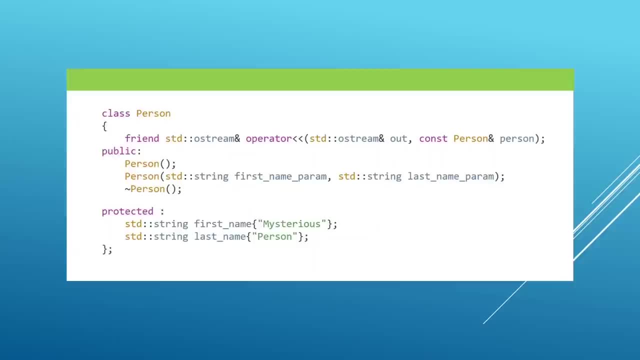 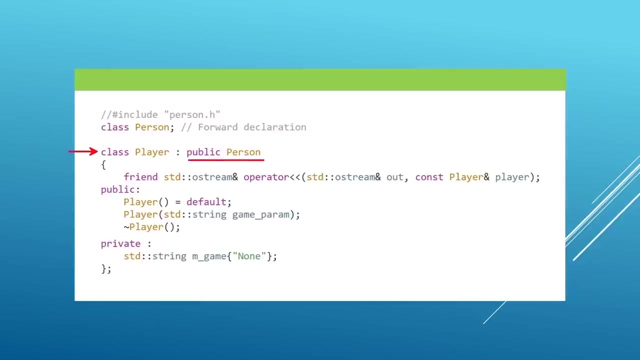 we will be able to modify these guys from a constructor of the derived class and we saw that that was impossible from the last lecture. but still we want to be able to use these from the outside of our derived class, which is person here. so we're going to still do public inheritance like from the last lecture, but now that our member variables in 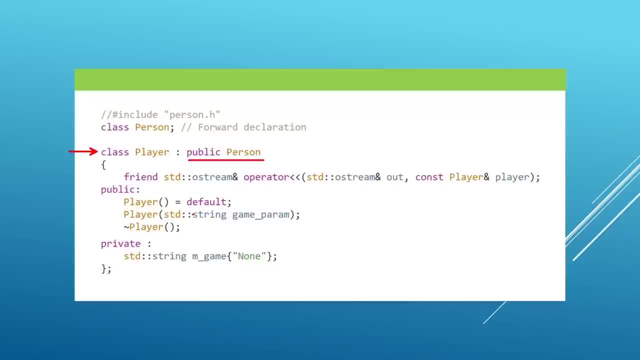 the base class are protected. we will have the ability to do whatever we want with them in the derived class. and when we say in the derived class, we mean from any method from the derived class. for example, we can go in our constructor here and then set data into the member. 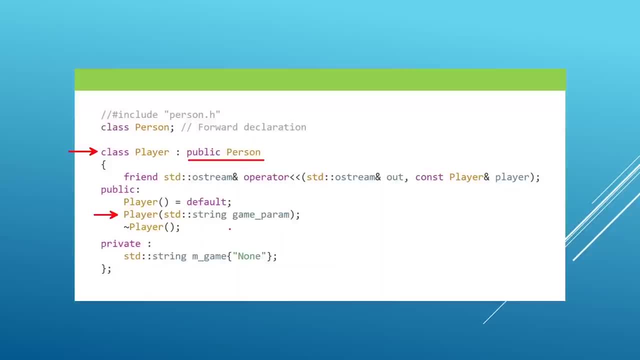 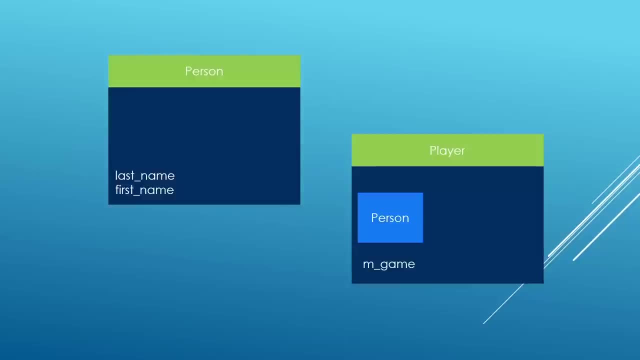 variables from the base class, and that's going to work, as we're going to see in a minute. now that you know this, we're going to head over to visual studio code and play with this a little more. okay again, our member variables from the base class are going to be protected. okay, so we can really say: 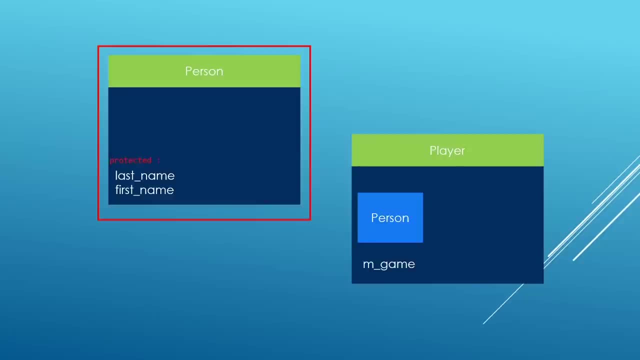 that here let's say protected, and at the moment we do this. they are going to be accessible and usable from a derived class. so from the derived class we will have the first name, for example. so from the derived class we will have our members baked in. we will have a last name and the first. 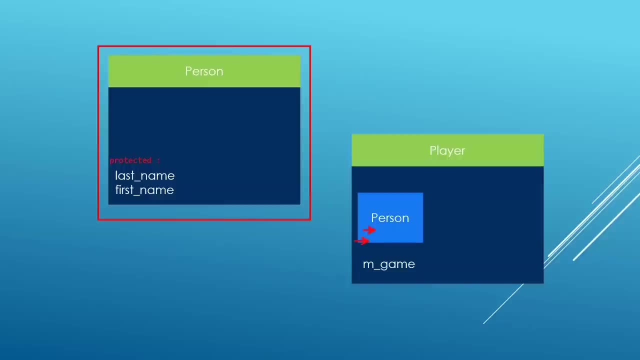 name and because they are protected in the base class and we are doing public inheritance, we will be able, for example, to set data into these member variables from a derived class, and that's going to be really cool. now that you know this, we're going to head over to visual studio code and play with. 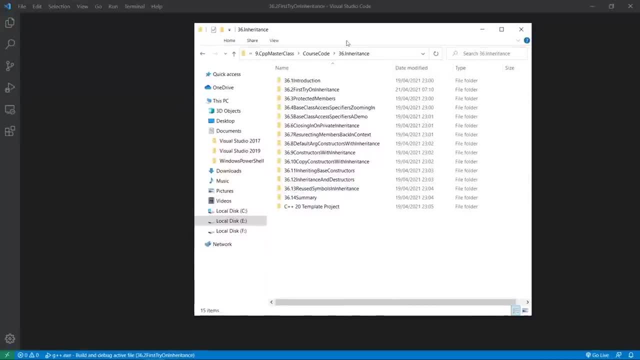 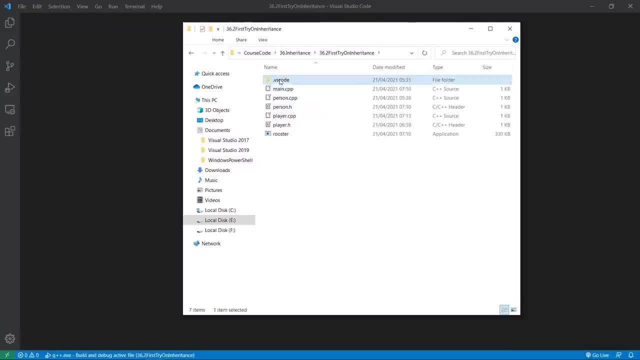 us a little more. okay, so here we are in our here we are in our working folder: the current project. we are going to have our protected members. we're going to grab the code from the last lecture and reuse that, because that's going to have our inheritance hierarchy already set up. we will 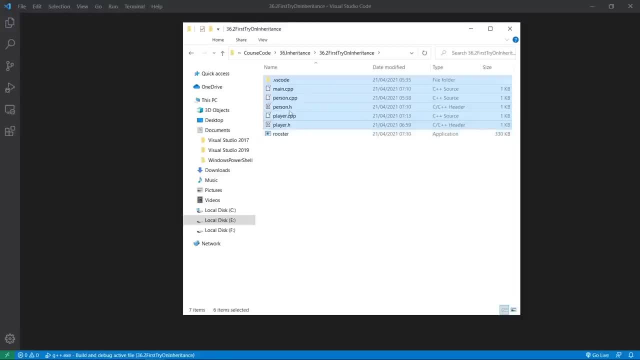 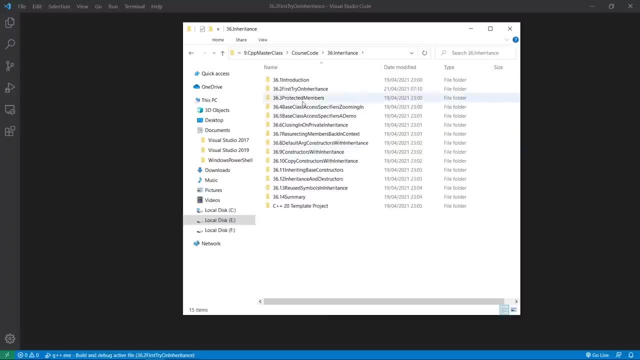 have our person and player class and we can reuse them. we will have our person and player classes and we will reuse them without needing to completely set them up from scratch. that's going to save us a few seconds, so we're going to put them in here and we are going to open this. 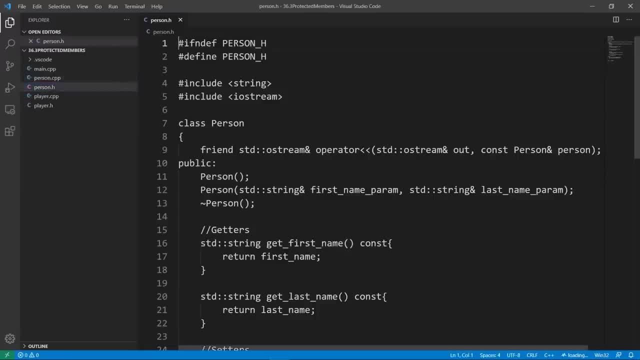 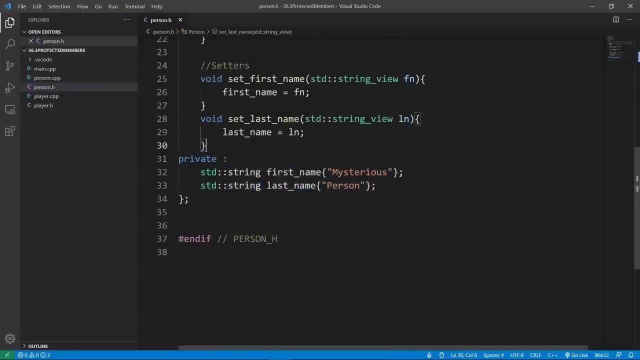 your studio code by dragging and dropping here and we will have our person class, which is going to be the base class. it's going to have our member variables, which are going to be private from the last lecture. we will have our player class, which is going to be inherited publicly from the player. 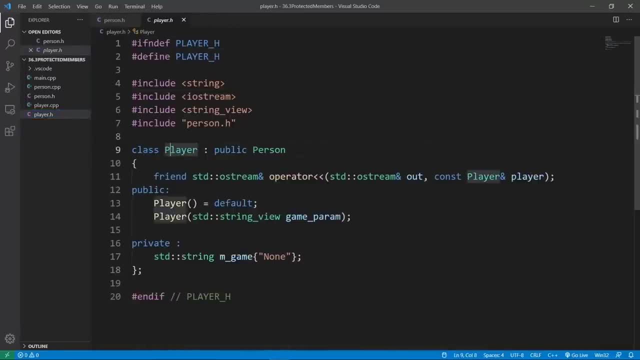 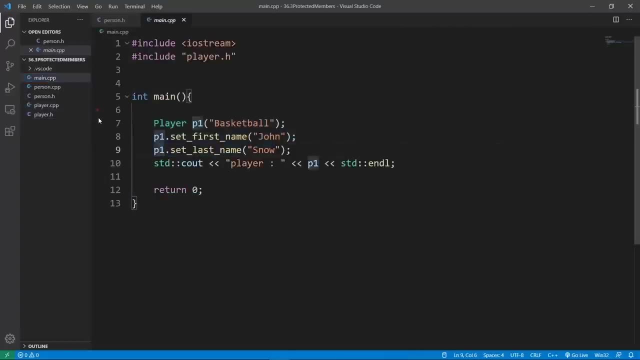 we will have our player class, which is going to be publicly inheriting from person, and we have our main cpp file which is going to set up a player object and try to use it, and we're going to see how this goes in this way. so what we want to do is to change the access specifier in the base class and make that. 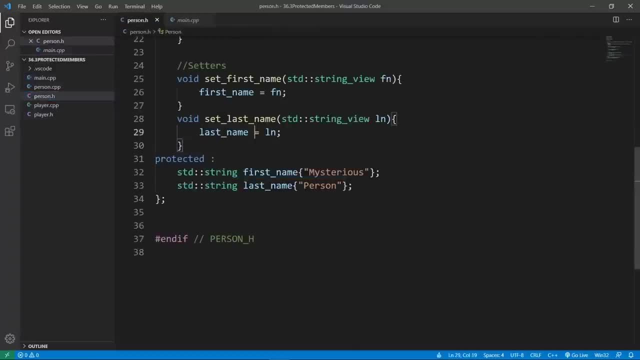 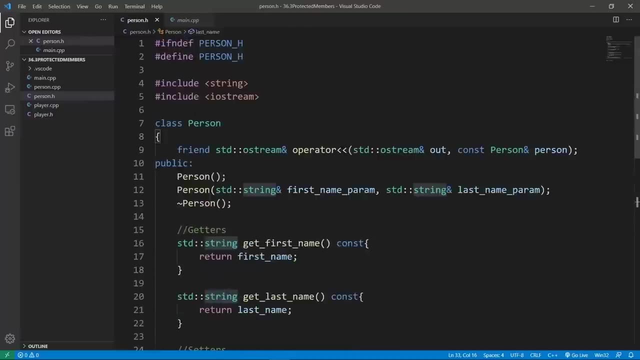 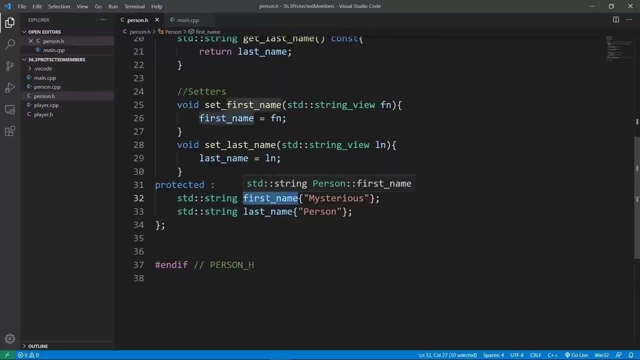 protected. we can do that. we can say protected, and this is going to change a few things about this class, what this is going to do. if you do public inheritance from this person class, you will have the ability to do whatever you want with these member variables from a derived class. 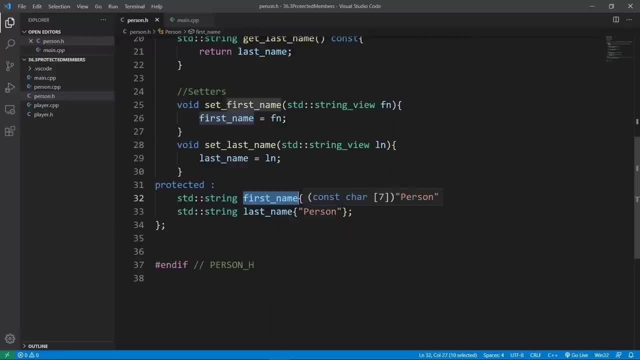 you will have the ability to write into these member variables and change the data that's going to be available in the base class that we have inside. you will also have the ability to read from them, and that's something we couldn't do from the last lecture, and this may come in handy. 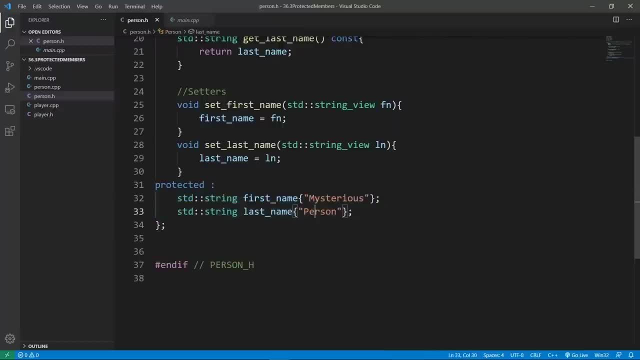 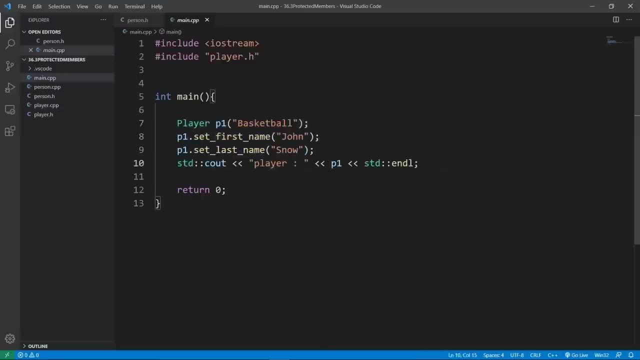 sometimes. another thing you should know is that these members are still not going to be accessible from the outside. so from the standpoint of the main function, for example here they are going to behave as if they are private because they want to be accessible from the outside. they will only be. 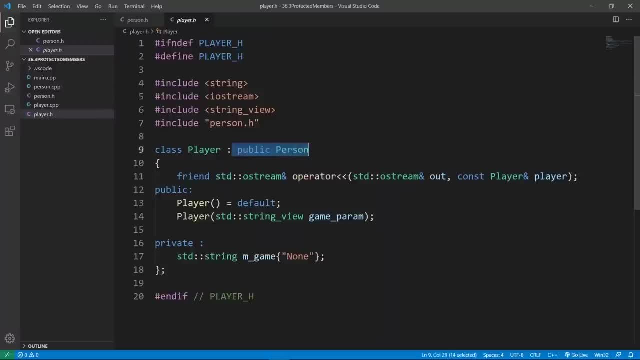 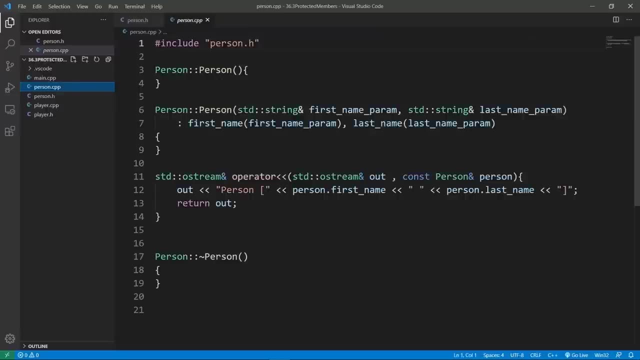 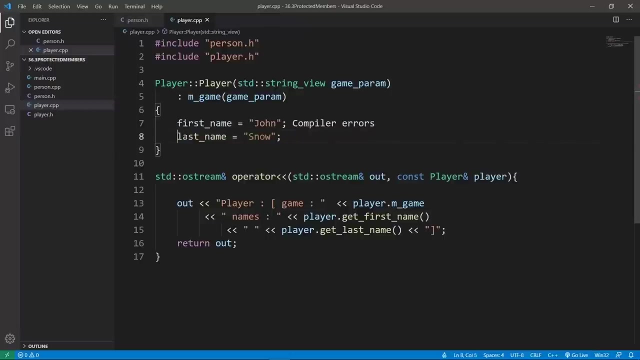 from derived classes that do public inheritance. this is really important to understand. now that we have this, we can really do all kinds of crazy things. for example, we can go in our constructor of player and comment what wasn't working from the last lecture and this is going to work now. 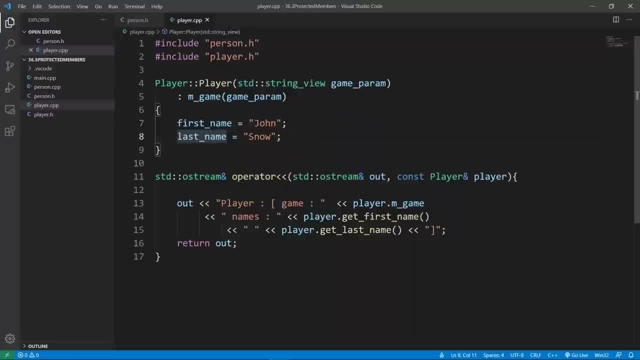 so let's uncomment this and we're going to see that the squiggly lines are going to go away. and if we build a player object using this constructor, we're going to see that we're going to have a john snow n, even if we don't set using the setters from the base class. so we can. 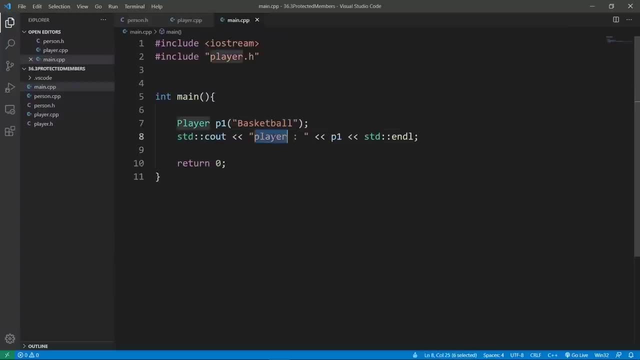 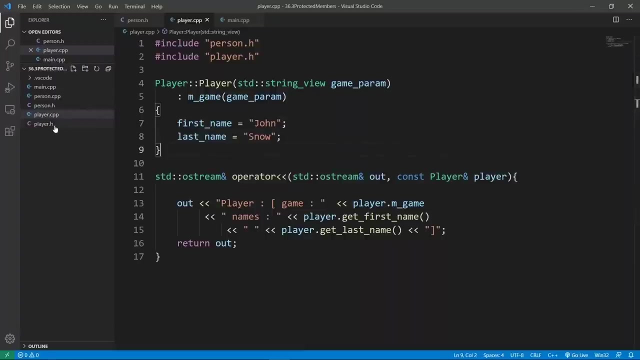 take these out and if we print information about this player, we're going to see the game to be basketball and the names are going to be john snow, because we are setting up this in the constructor of player. that's no longer. that's no longer going to be the data we get from the 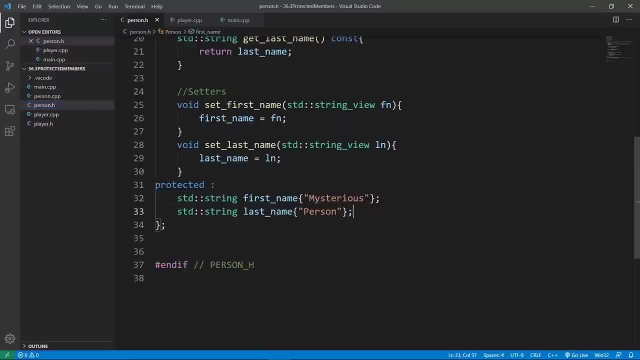 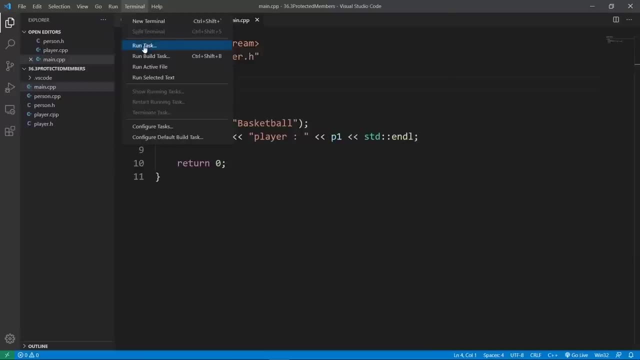 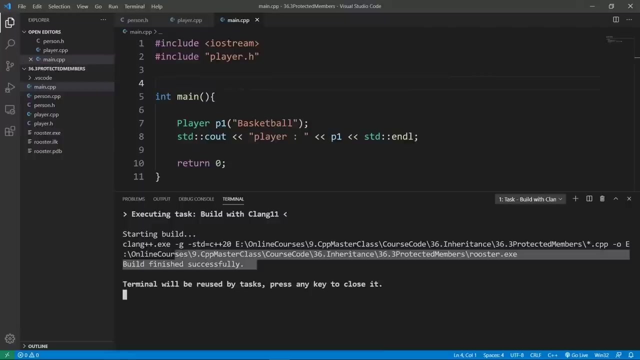 constructor of a person object, which was here in the base class. let's try to build and run this program so that you can really see this. i just used clan here, but it is also going to work. no big deal here. the build is going to be good. we can clear and bring up a powershell window we can use to run. 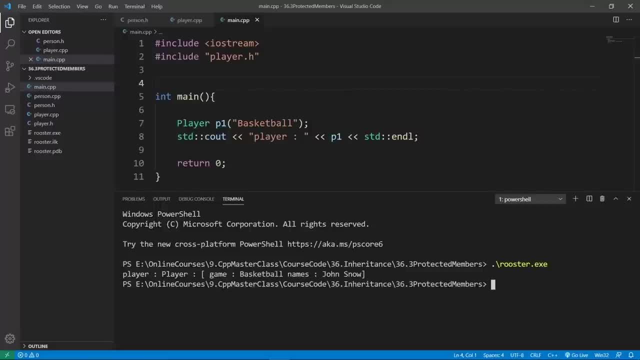 this program. we're going to say rooster and you're going to see that player is going to be the heaven. the information, the game is going to be bastard ball, the names are going to be john snow and we are setting this data from a derived class and we have the ability to do this because these 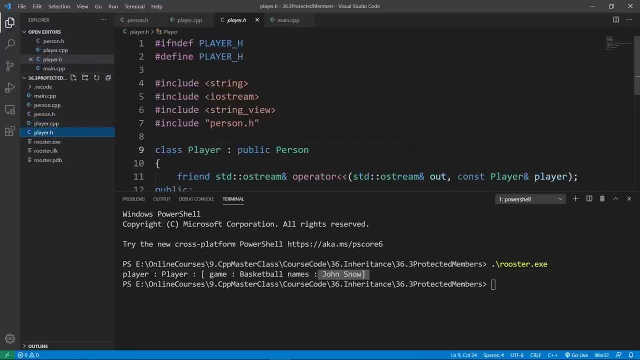 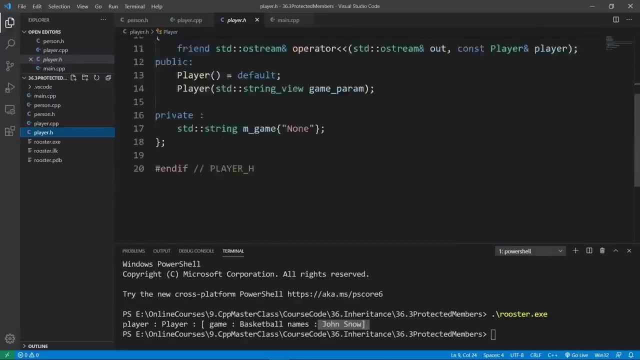 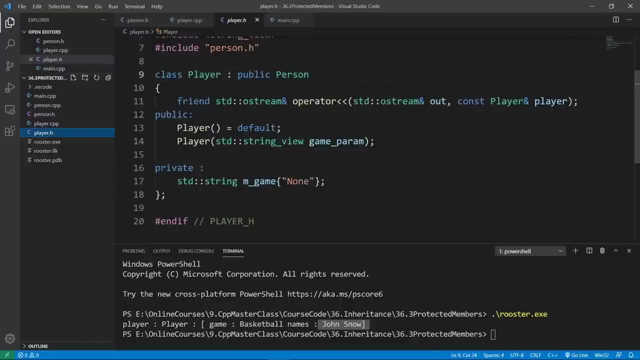 members are now protected in the base class, so they are accessible and usable from a derived class. now that we have this ability, we can really change how our class, at least the derived class, works. we're going to change the it to have two more parameters and we're going to pass the first name and the last name. 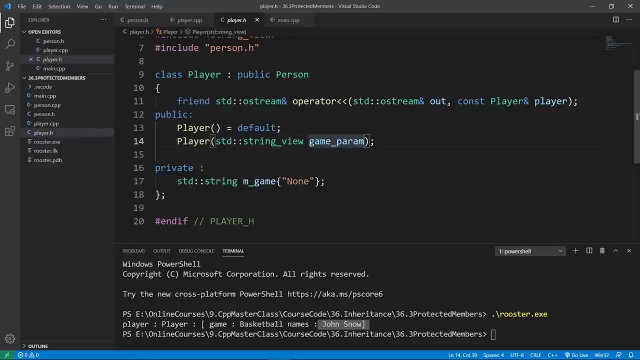 and pass this data back into the base class by setting the data in the body of the constructor. this is going to work, so let's add our parameters. we're going to say std string view, and this is going to be first name param and we're going to put in another one which is 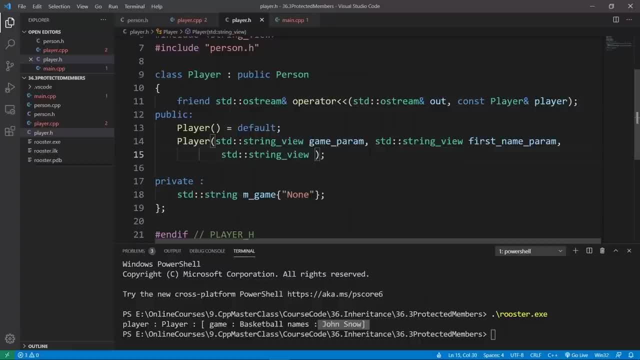 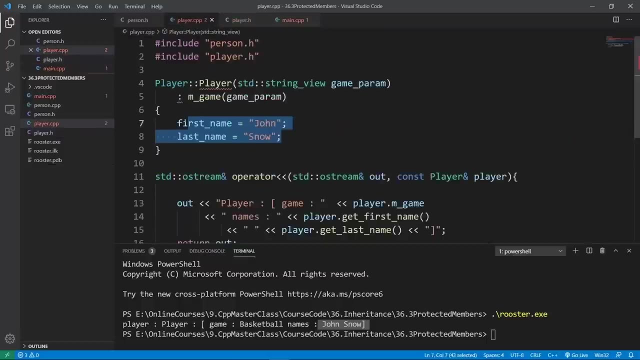 going to also be a string view parameter and it's going to be last name parameter. we can say that and we're going to hop over in our implementation. let's grab what we just added, because we will need to put that in our cpp file. we are going to go in playercpp and we're going. 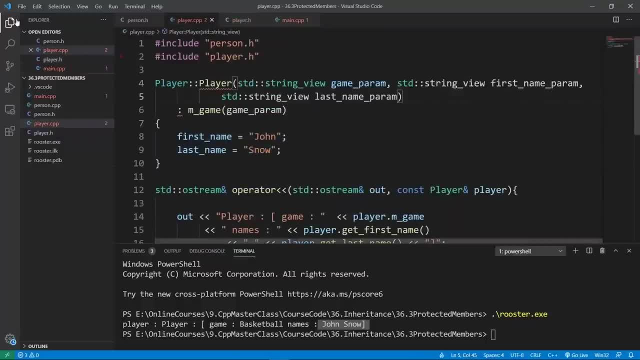 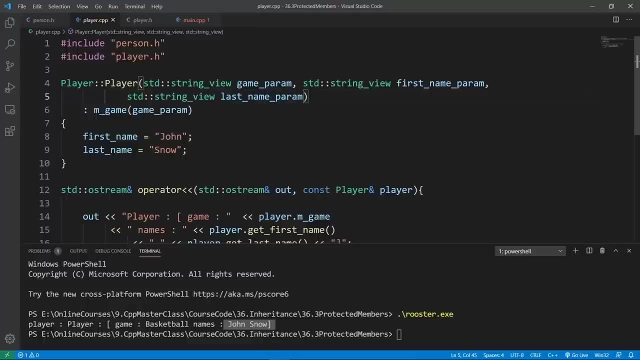 to add this data. we're going to put that here. we can close the left side bar to have some more breathing room, and then we're going to not do an initializer list here, because this is really going to be useless. we are changing data in the body of the constructor, so we're going to add this data to. 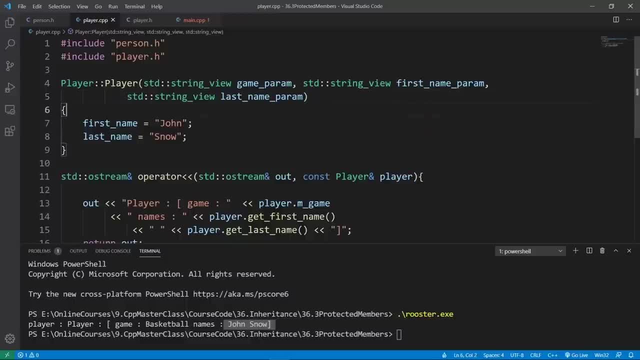 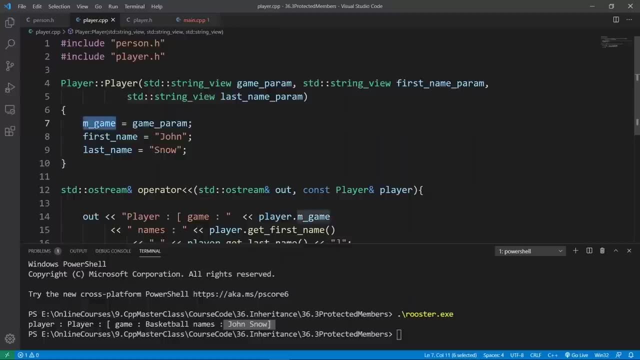 our cpp file anyway. so what we can do is say game param or game, and we're going to say game param. i am really sorry. i am not following the same convention for the naming of my member variables, but we can change this later. so let's say first name. we are going to pass in first name param. 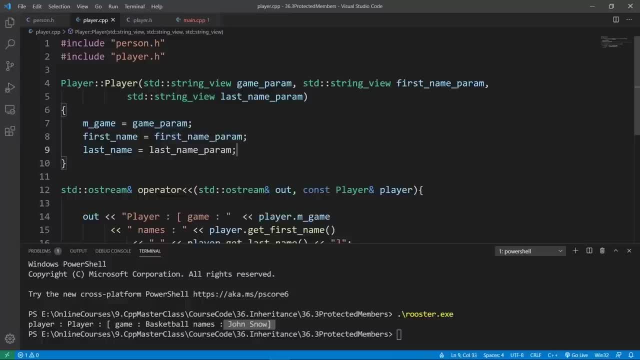 and for the last name, we're going to say last name, param, and that's going to do. now we have the ability to go in the main cpp file and create a new cpp file and we're going to create a new cpp file and we're going to get player objects and specify the first name and the last name and this is going. 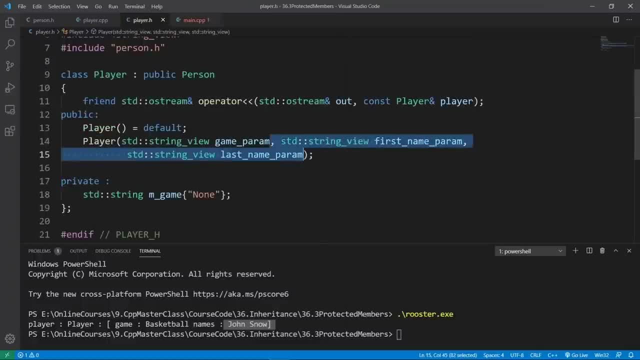 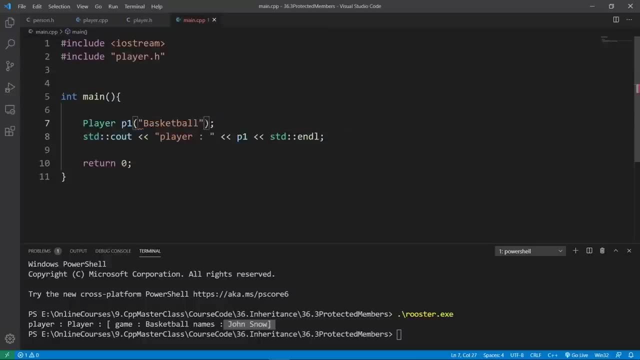 to be much more flexible. so let's go back to the constructor and see the order of our parameters game: first name, last name. so we can come here and say first name is going to be john and the last name is going to be snow, and if we build and run, we're going to see the information printed out. 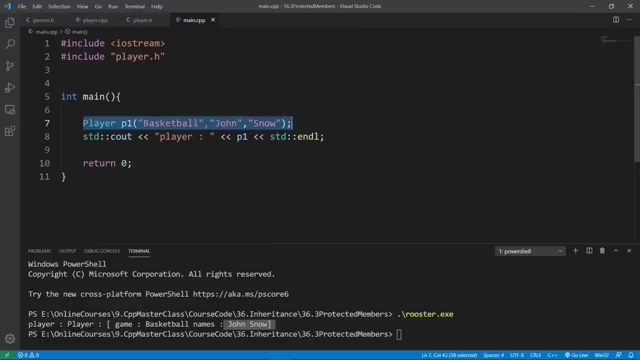 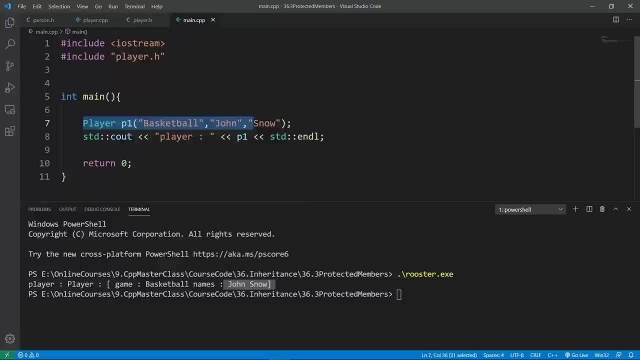 here and now we have the flexibility to be able to specify this in our cpp file and we're going to go back to the constructor, and this is going to make the job of building our objects much easier, and we can forward this data back into the base class using the protected mechanism that we just 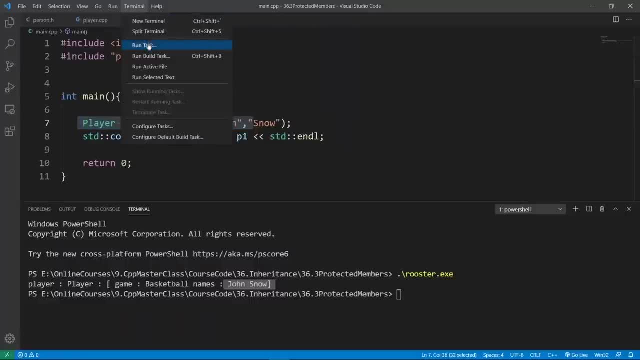 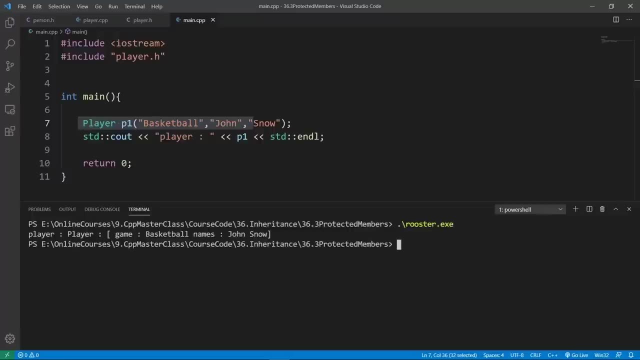 learned about in this lecture and this is really cool. so let's build. we're going to pass this through gcc and the world is going to be good. we can clear and run rooster. we're going to see that the data is passed back to the base class and this is working really well. okay, so this is really. 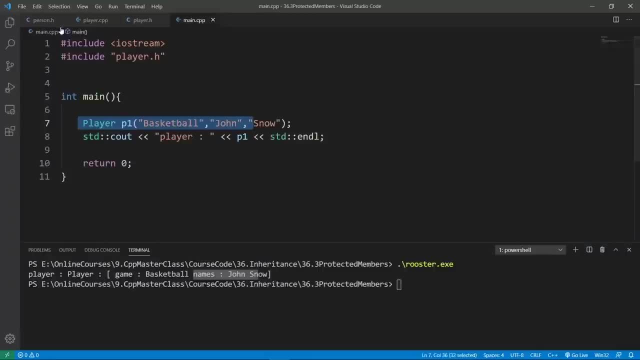 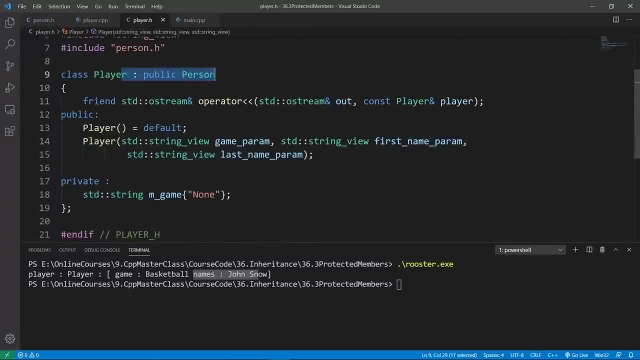 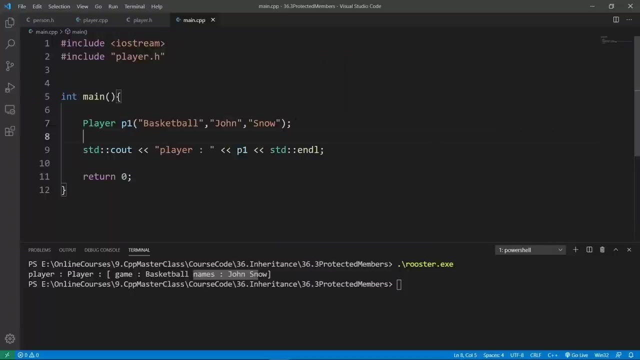 all i wanted you to see in this lecture. we can set up protected member variables and they are going to be accessible and usable from any derived class that does public inheritance. but they want to be accessible from the outside. so if you try and, for example, say p1 and say 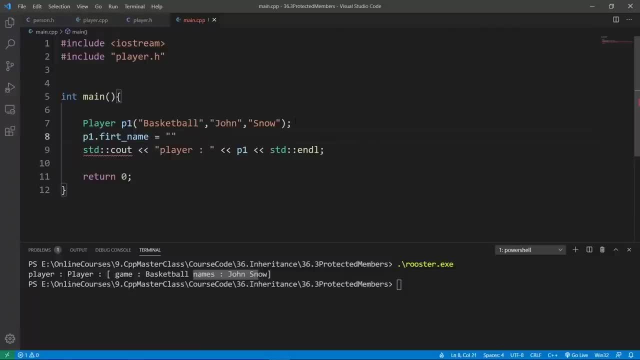 first name and try to change that to something else. let's say daniel, for example. you're going to have compiler errors because this is not going to work, so let's try and build and show you the compiler error. okay, so protected members are not accessible from the outside. 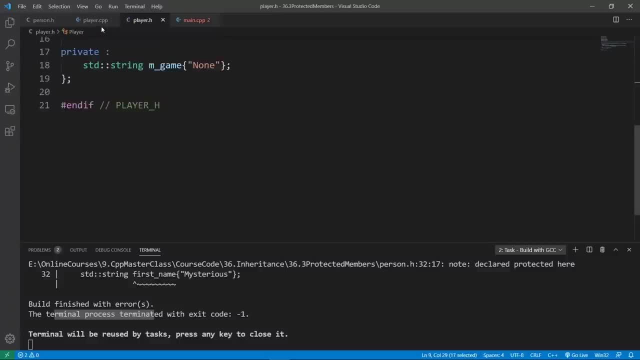 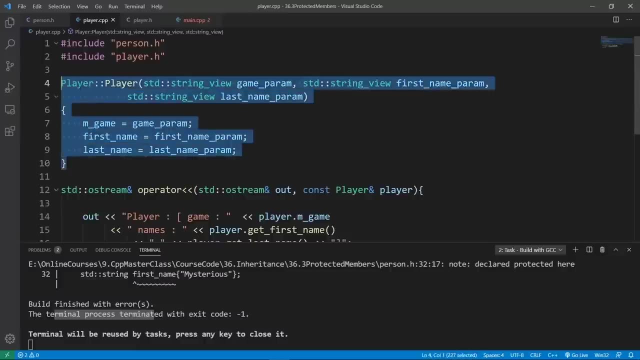 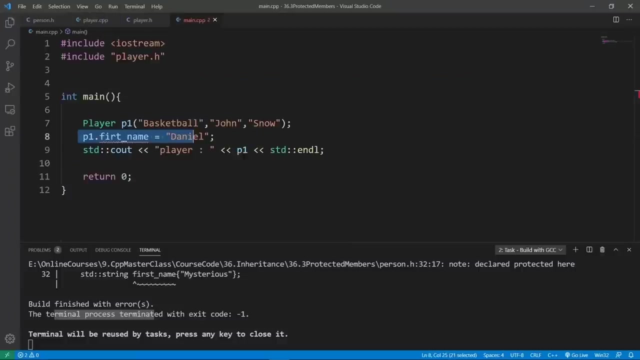 they will be just accessible from derived classes or, to be more specific, they are going to be accessible from the members of the derived class, and by members i mean member functions, because that's where you will be accessing and modifying stuff. so let's go back to the main cpp file and 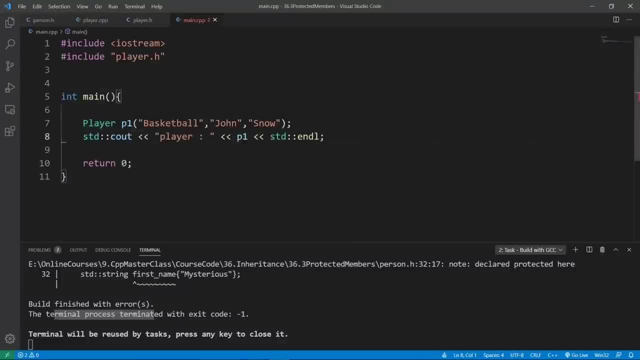 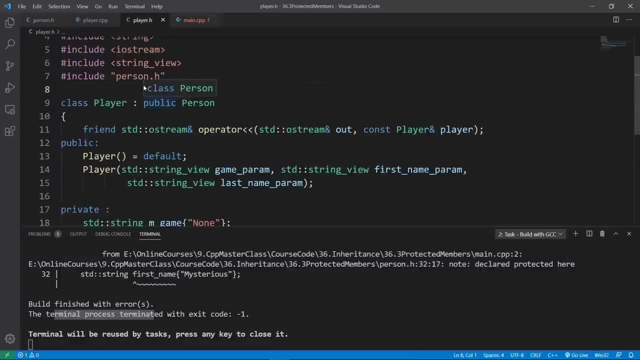 remove this and this is really all i wanted to share with you and i hope you enjoyed the video. hope you found this lecture interesting. We are going to stop here in this one, and in the next one we're going to zoom in on the syntax here we are using to derive from other classes. We just 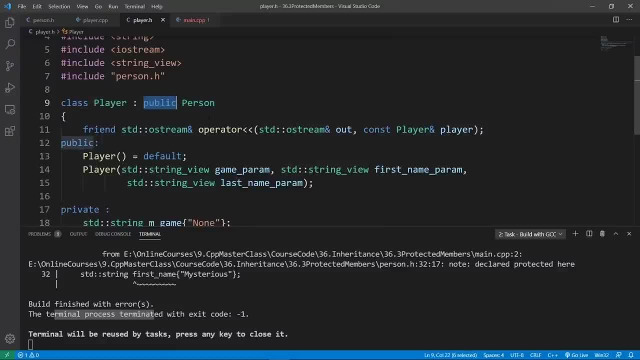 did public inheritance here, but in the next lecture we're going to see that it is possible to actually do protected and private inheritance, and we're going to see what this means in the next lecture. So go ahead and finish up here and meet me there. In this lecture we're going to 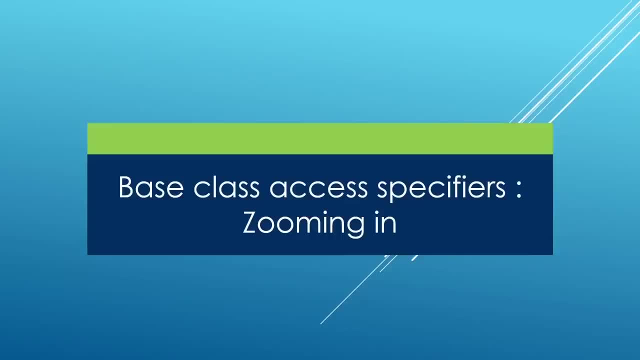 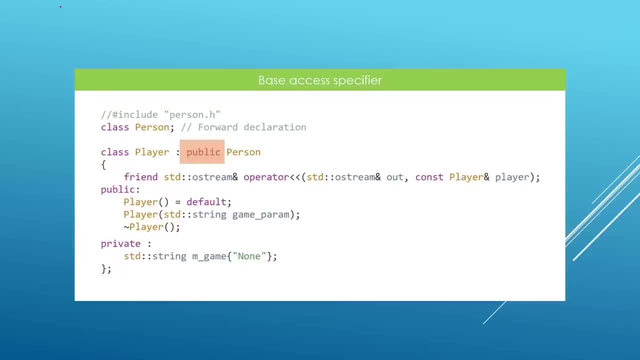 learn about base class access specifiers and, in case you didn't know, we have been using base class access specifiers in this chapter all along. and to really understand this, let's look at our player class, which is inheriting from person, and we are doing public inheritance, The public keyword here. 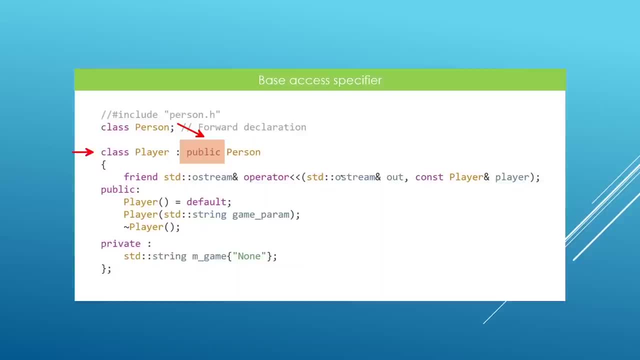 is a base class access specifier and it is going to control how accessible are base class members from the public class. So let's go ahead and see what we're going to do here. So let's go ahead and see what we're going to do here. So let's go ahead and see what we're going to do here. So 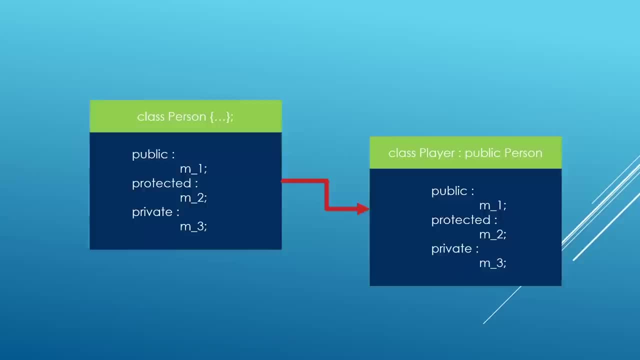 from a derived class and we have three options. Okay, so if we do public inheritance, like we see here in our player class, anything that is public in the base class is also going to be public. You see, m1 here is also public in the derived class. Anything that is protected is going to stay. 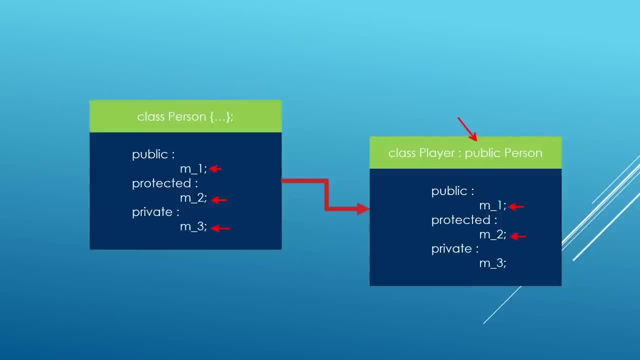 protected, and anything that is private in the base class is also going to stay private in the derived class. Try and take a moment to see what we're going to do here. So let's go ahead and see what we're going to do here. So let's go ahead and see what we're going to do here. So let's go ahead. 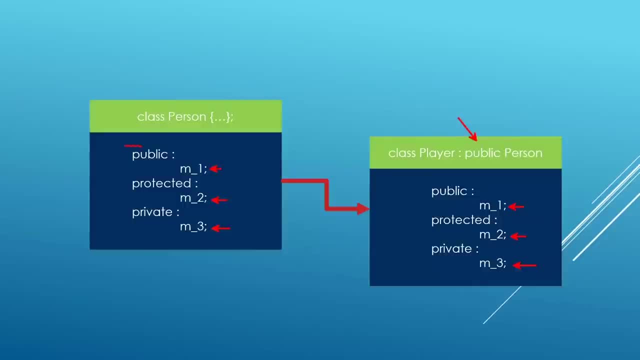 to look at this again. The member access specifiers we have in the base class are going to stay intact if we do public inheritance Again. anything that is public in base is going to be public in derived. Anything that is protected in base is going to be protected in derived, and anything that is private 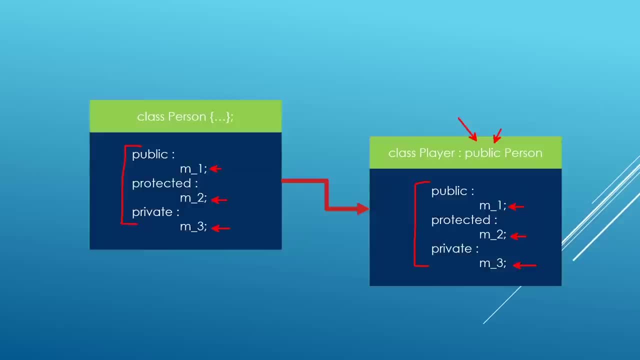 in base is going to be private in derived. This is one kind of inheritance we can do in C++. but we can also do protected inheritance and the syntax to do that. you just use the protected keyword. here You say class player, colon, colon and specify that you want to do protected inheritance. 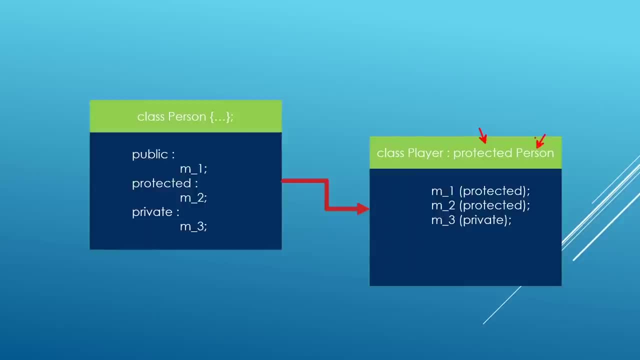 and then you specify the base class you want to inherit. from The moment you do this, anything that is public in the base class is going to be protected in the derived class. Anything that is protected is going to stay protected. Anything that is private is going to be private, and in one way you can see that we can use these. 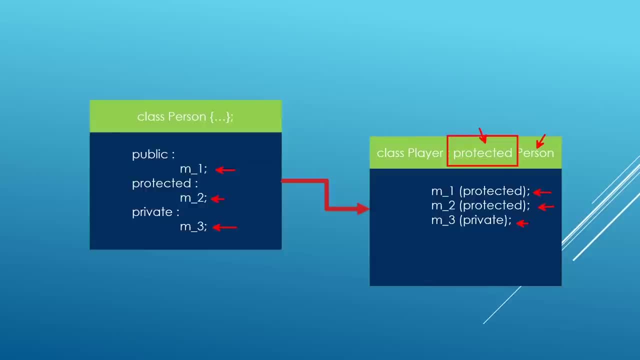 base class access specifiers to constrain the access specifier in derived class. but we can't make the access specifiers in derived class more relaxed. We can only make things more constrained or more restricted. For example, the m1 member variable was public but now we have made it become. 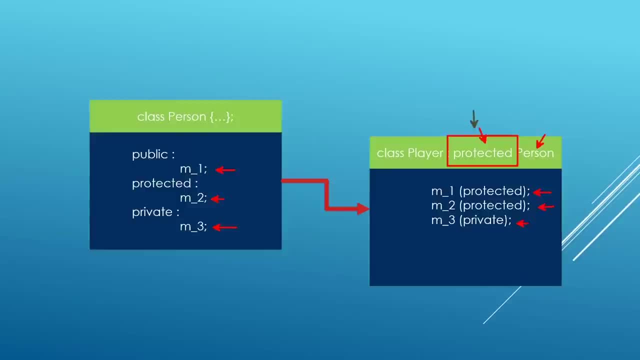 protected By using the protected base access specifier here. Okay, so now you know that we can do public and protected inheritance, but it is also possible to do private inheritance and you do that by using a private base class access specifier. The moment you do this, anything that is public in the base 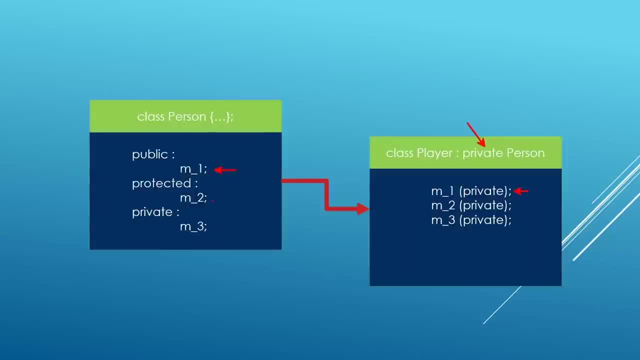 class is going to become private in the derived class. Anything that is protected in the base class is going to become private in the derived class. Anything that is private is going to stay private in the derived class. and again you see that this is going to constrain things. Things that were public are now private in derived, and we can't. 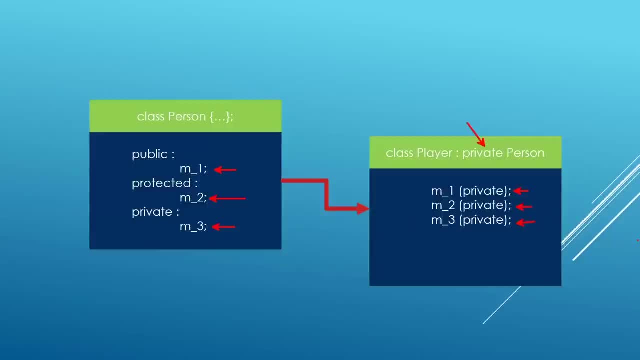 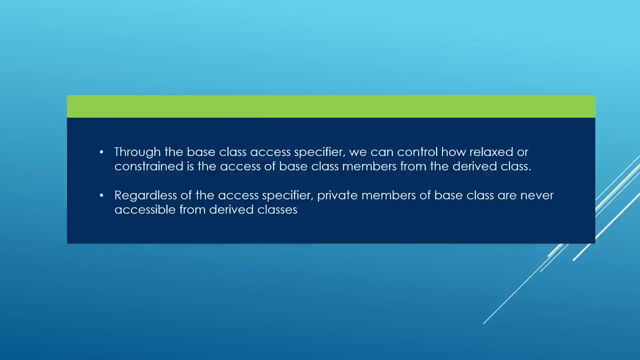 really do anything with them from any other class that might derive from our player class. So this is the setup we have. Okay, to sum this up: through the base class access specifier, we can control how relaxed or constrained is the access to base class members. 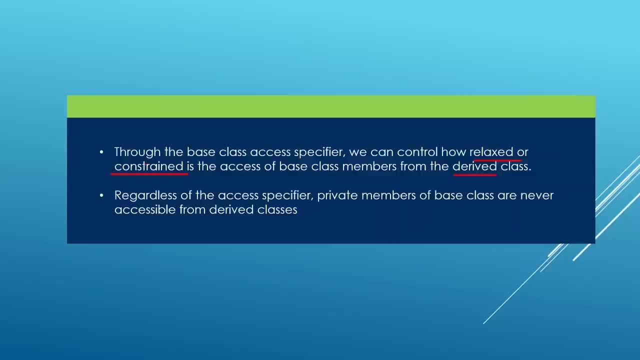 From the derived class, and this is really important to understand. If you want to say as relaxed as they are in the base class, you can use public inheritance. If you want to constrain a little bit, you can use protected inheritance, and things are going to be inherited as protected, except for the private data in the base class. If you want things to be super constrained, you can use the private inheritance that we just learned about and everything in your derived class is going to be private. 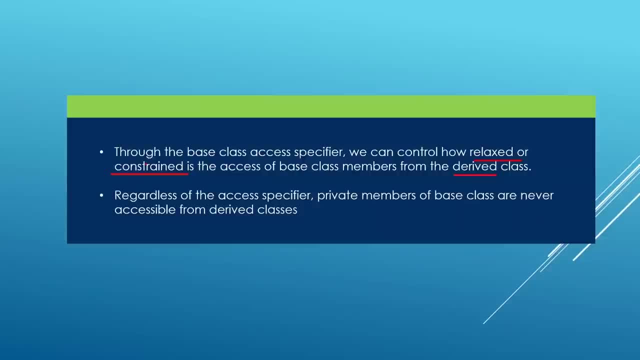 And you can use this if it makes sense for the application you are designing, And you can use these kinds of features if they make sense for whatever application you are designing with C++. One thing you should know, though, is that, regardless of the base class access specifier we use, private members of the base class can never be accessible from a derived. 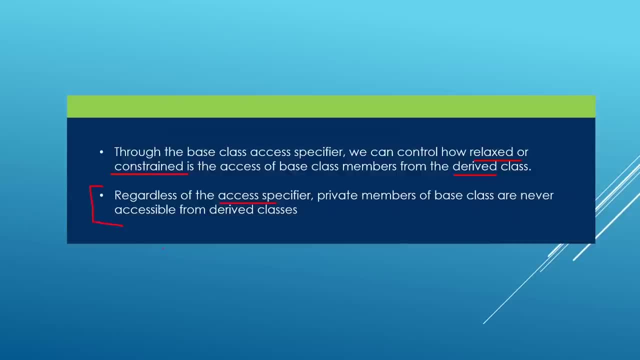 class. So anything that is private is going to stay private and you have no way to relax things a little bit. That's not going to work. You should really know this. Now that you know these kinds of inheritances we can do in C++, we're going to head over to the 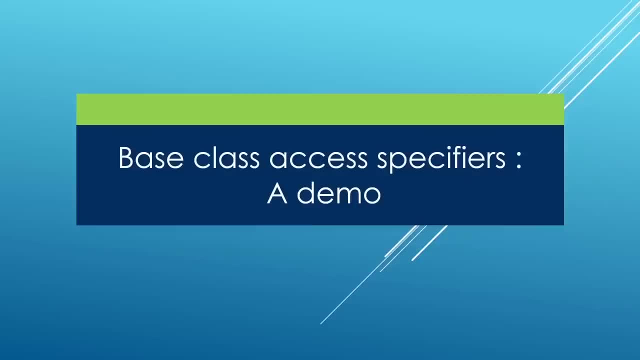 next lecture and play with them a little more. In this lecture we're going to play with the base class access specifiers we learned about in the last lecture. In other words, we're going to play with public, protected and private inheritance in Visual Studio Code. So let's. 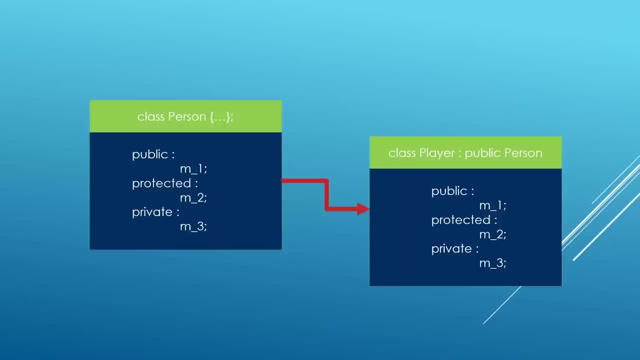 review a little bit what we talked about in the last lecture. We said that we can have public inheritance and the syntax to do that is what you see here And the moment you do this, what was public in the base class is going to be public in the derived class. What was protected. 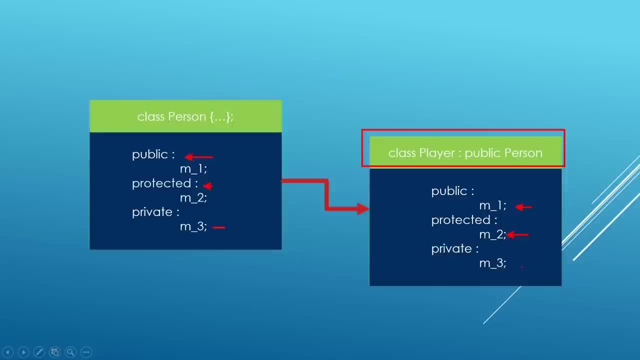 is going to stay protected. What was private is going to become private in the derived class. In other words, public inheritance is really not going to change the accessibility of the member variables we have in the base class. We're going to inherit the data as it was, with the same access. 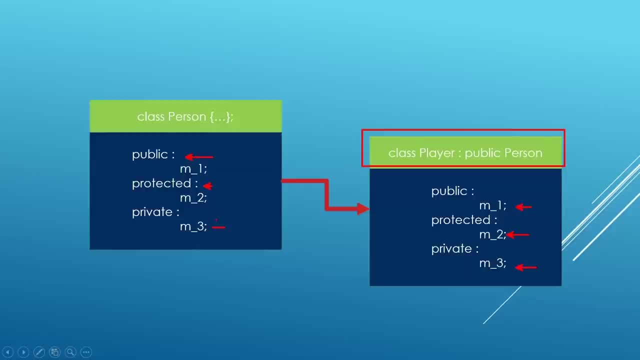 level we had in the base class. This is a defining feature of public inheritance. in C++ We can also do protected inheritance and what this is going to do is to make protected the highest access level we can have in the derived class. So anything that was public in the base class is going to 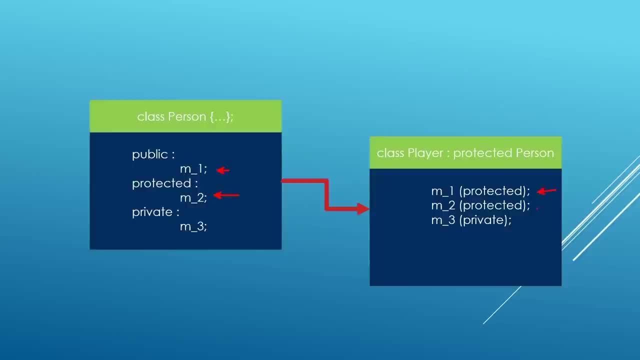 become protected. Anything that was protected is going to stay protected because that's the highest level it can do now, And anything that was private base class is going to be private in the derived class. we say private in the sense that it is going to be private to the base class, so you can't really use m3 from the player class in this case. 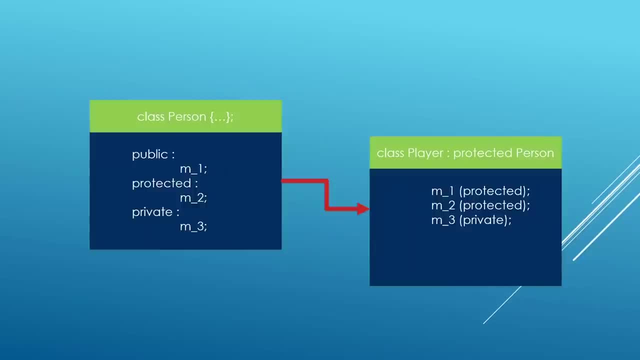 if you're trying to do that, you're going to get a compiler error. okay, we can also do private inheritance, and the syntax to do that is what you see here and now. private is going to be the highest level we can do in the player class in terms of the members that we got from the base. 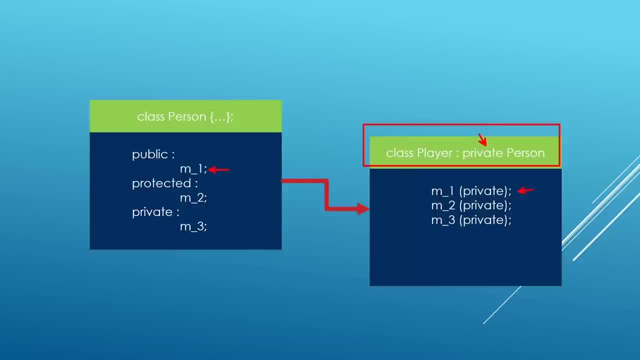 class. so anything that was public is going to become private, anything that was protected is going to become private. anything that was private to the base class is going to stay private to the base class. this is what we mean here. but now m1 and m2 just became public to the player class. if 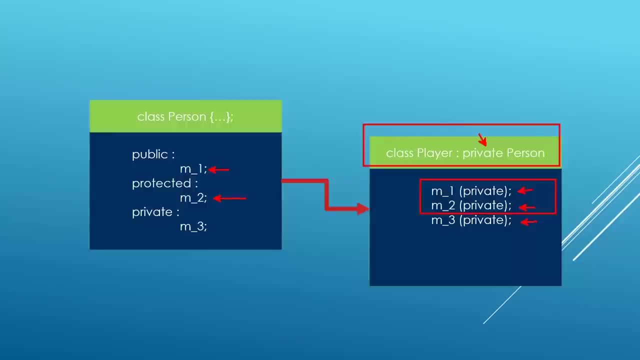 anybody else tries to derive or inherit from a player. these things are not going to be accessible and this is in some way the player class being selfish. it is saying i am going to get everything i can from my parent class or my base class, but i am going to make it all mine. nobody else can take this, and this is the kind. 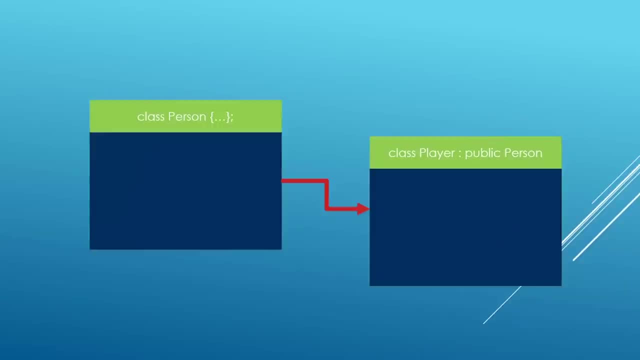 of setup we can achieve with private inheritance. okay, so now that we have this in mind, we're going to play with us in visual studio code. we're going to set up a bunch of classes. we're going to set up a personal class we're going to be inheriting from. we are going to set 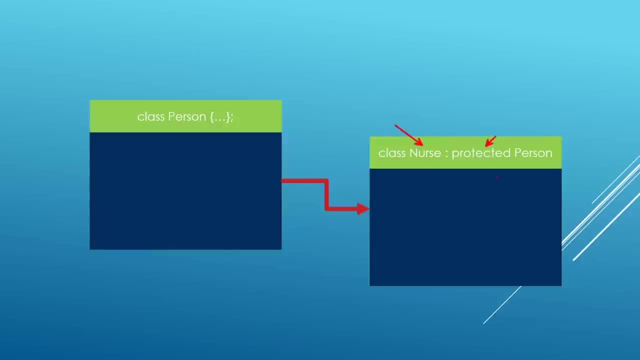 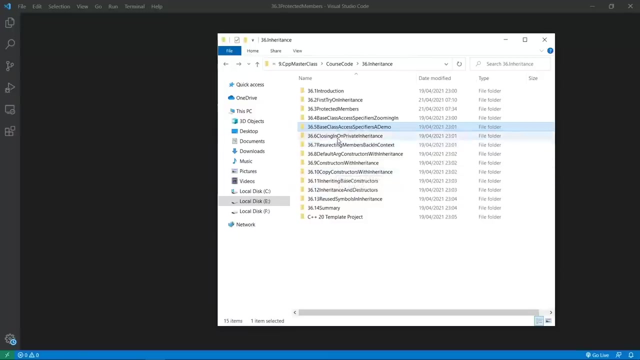 up a nurse class which is going to do protected inheritance, and we're going to set up an engineer class which is going to do private inheritance, and we're going to really play with us and see how this plays out in real c plus plus code. so let's do this. here we are in our working folder, the 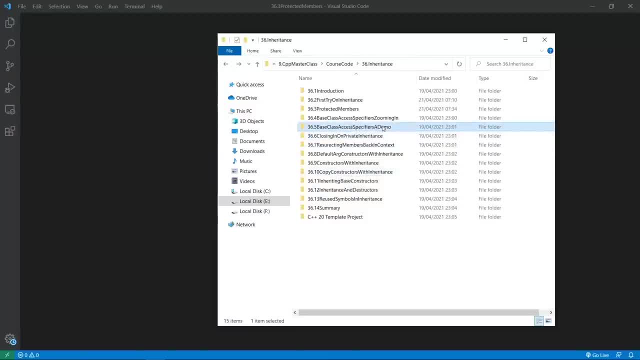 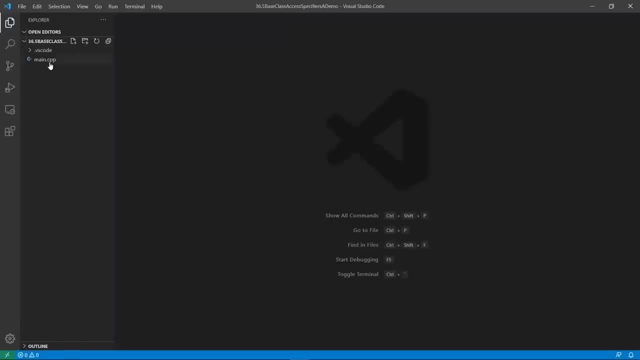 current project is base access specifier- a demo. we're going to do a demo on this, but before we do that, we're going to grab our template files and put them in place and we are going to open this little guy in visual studio code by dragging and dropping here. this is going to give us a good starting point. we're going to 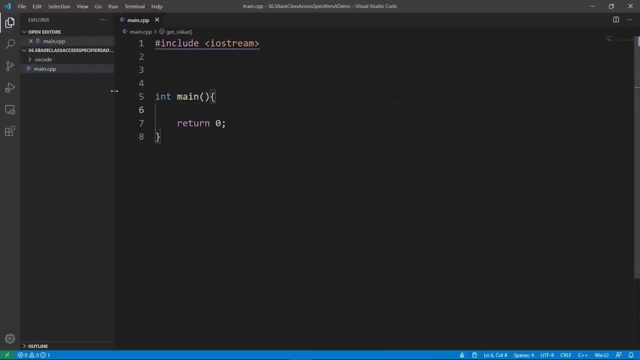 have our main cpp file. we're going to clean it up and we're going to set up our base class, which is going to be the person class. so let's put this in from scratch. we're going to add our files, we're going to say person h and we're going to say personcpp. we are going to hop over in our header. 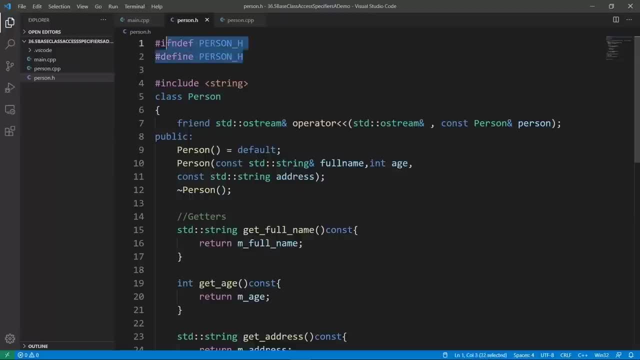 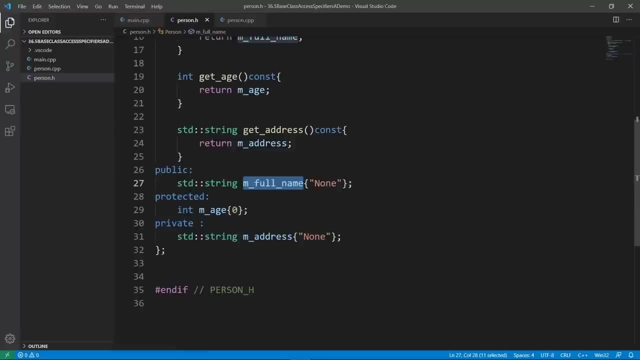 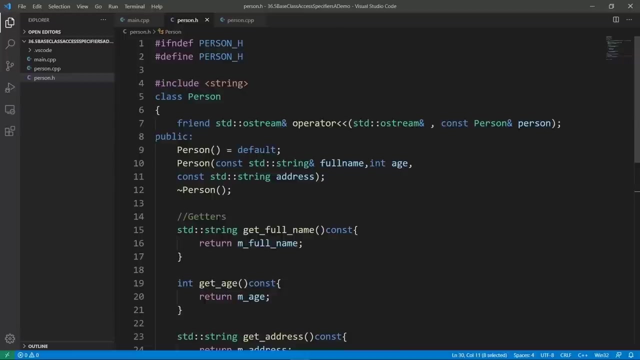 file and put in our code. nothing special so far. we have an include guard, we have our person class. it has a bunch of member variables. we have the full name, which is public, we have the age, which is protected, and we have the address, which is private, to this class. here. this is going to be our starting point. 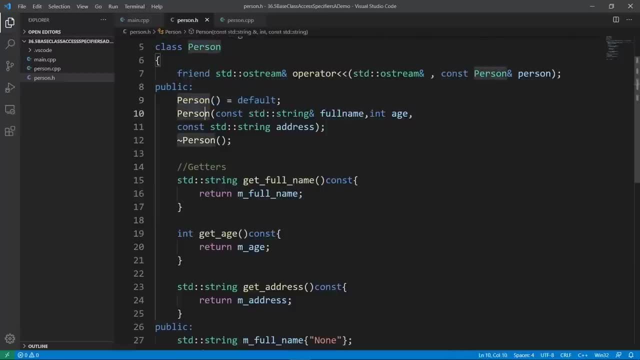 we also have a bunch of constructors. we have a default one. we also have another one which is going to take all the data we can use to construct a person object, and here we are passing string by reference. i think we can fix this and pass the string view. this is going to be better. 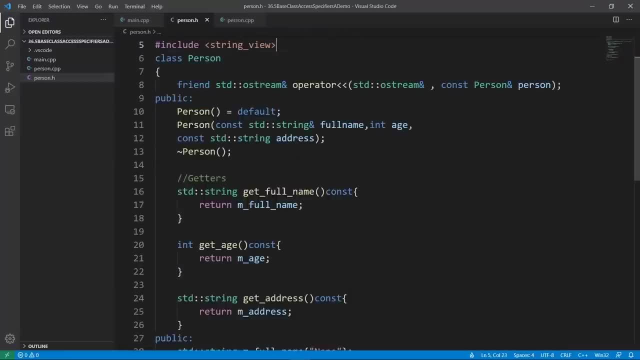 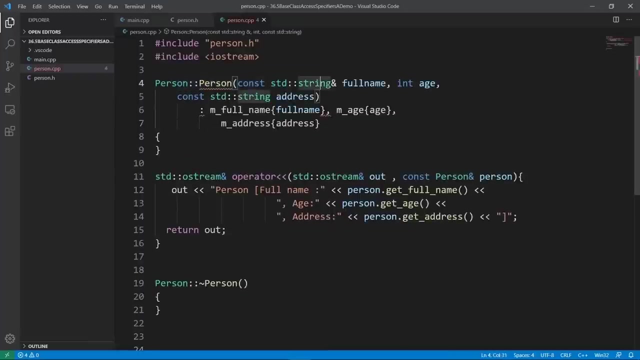 let's say string view, and we're going to change the first parameter here to be an std string view by value. this is going to be much better. okay, we have our class. we can hop over in the cpp file and put in our implementation. we are going to change the constructor a little bit and make 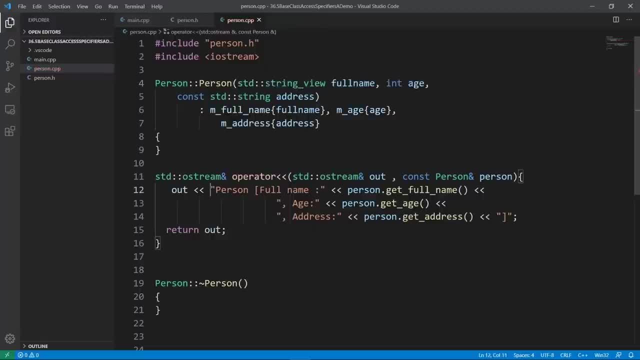 sure we are taking an std string view by value and if you wanted to type all this code, you can get it from the resource section of this lecture. i am going to attach all the source code and you can download and use this however you want to really make your learning experience. 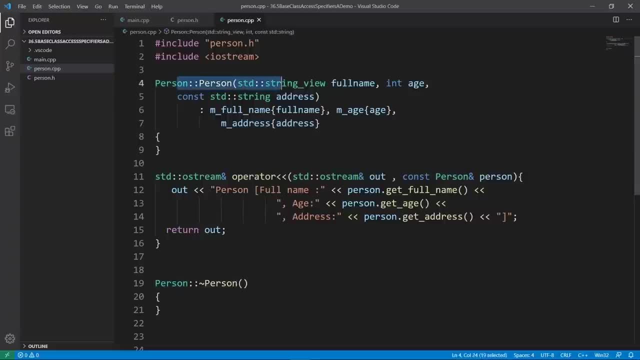 as pleasant as possible. so we have our constructor here. it is going to forward the data into our member variables. the full name is going to go into our full name member variable, we're going to grab the age and the address and we're going to store all this information. we also have an output. 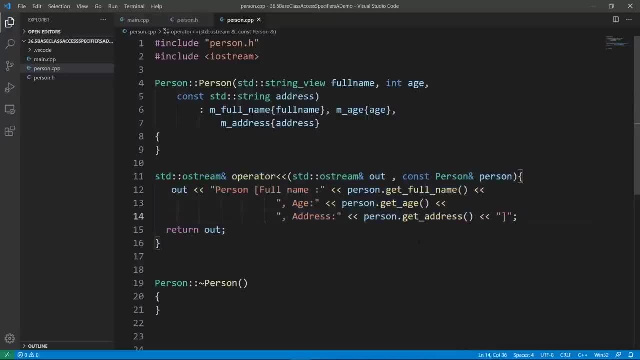 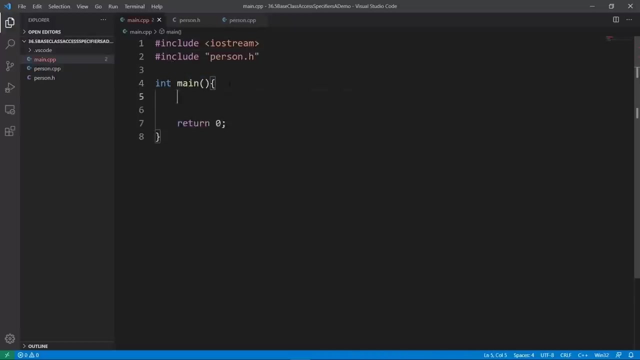 stream operator which is going to be printing all this information here. it is going to go through the getters because we have a person object passed as a parameter here and this is going to work. we can go in the main cpp file and include our person class and create an object of it. we can do something like person person one and we can pass the data. 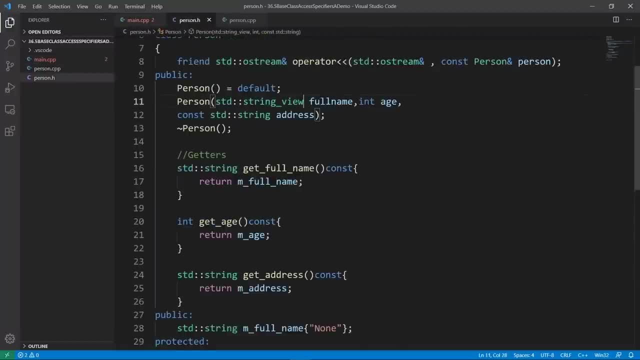 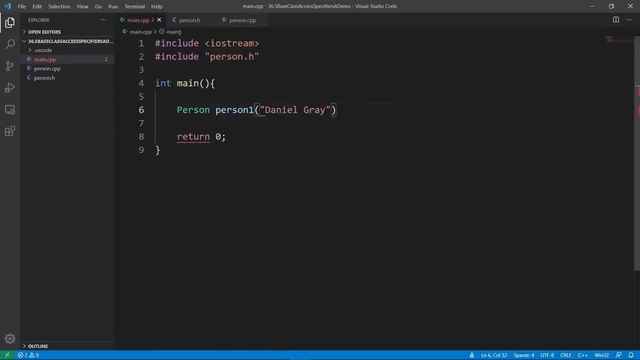 that our constructor expects we can pass in the full name, the age and the address. so let's do that. we're going to say the full name daniel gray, why not? and the age is going to be 26, seven. we can put in whatever we want. and we're going to put in the address. we're going to say: 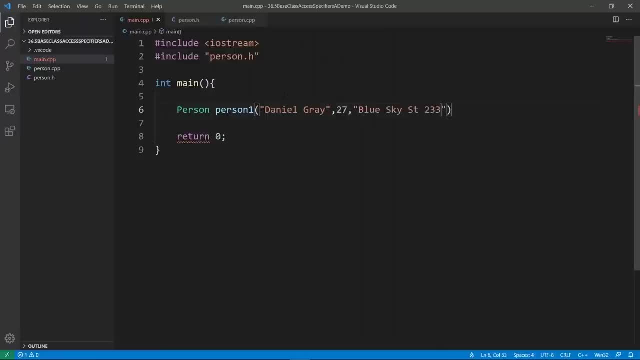 blue sky street. you can say two, three, three, for example, and say the number of the house to be 56, why not? this is a possible address for a person, so we can say person one. or we can use htdc out to print this out, because we have an output stream operator for our person class. 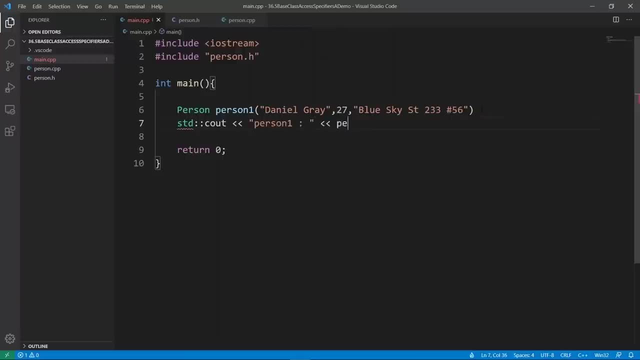 we can do this. we're going to say person one and we're going to put him out, and if we're going to run this program, we're going to see that this is going to work, hopefully. and we have a problem because we don't have a semicolon at the end of line 6 here. let's fix that. 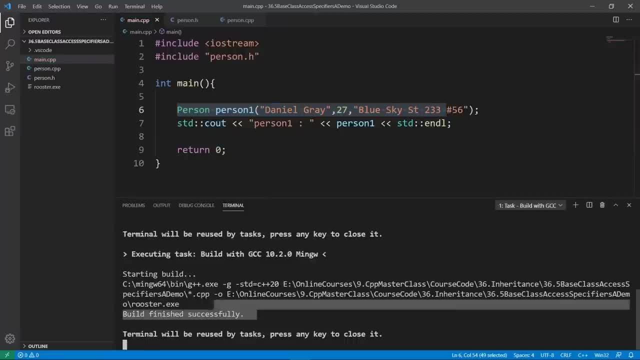 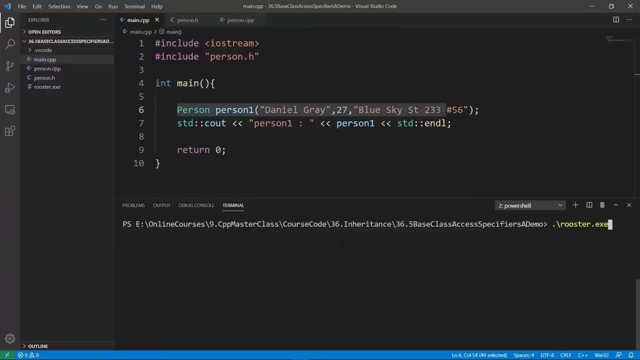 we're going to run this task, to build with gcc. the build is going to be good. we can bring up a powershell window and we're going to use this to run our program. if we say rooster, we're going to see that we have the person printed down. the full name is daniel gray, the age is 27. the address is: 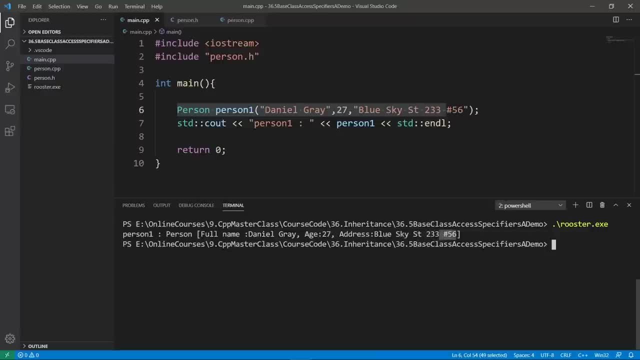 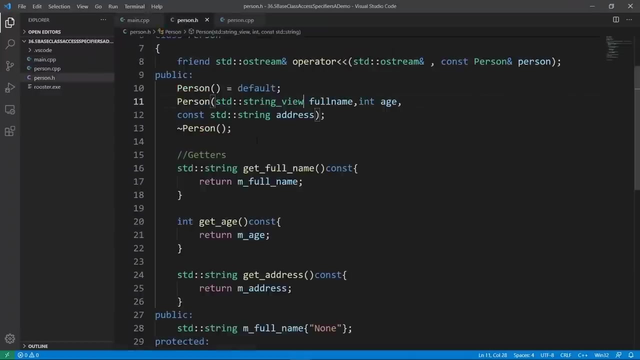 street 233 and the number of the house is 56. so this is a possible implementation for the person class. but we are really not interested in setting up a person class and doing things with that. we are interested in inheriting from the person class and learn about different kinds of base class. 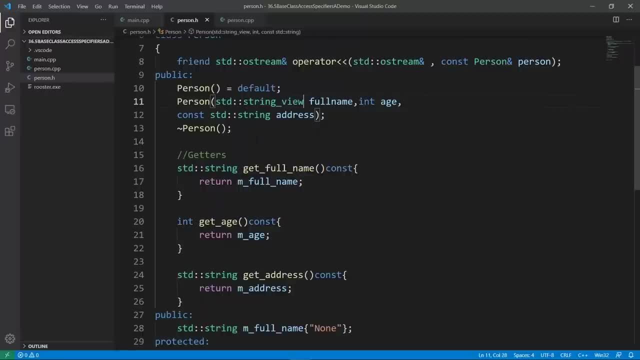 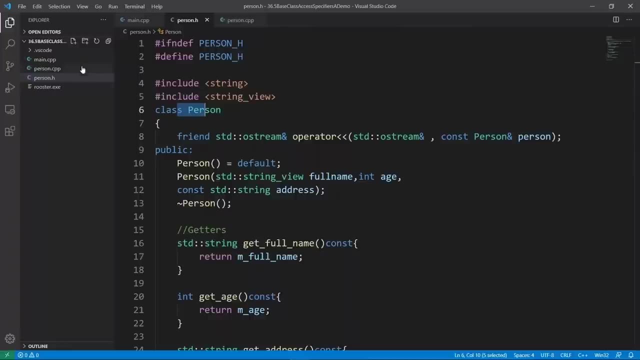 access specifiers. we can do so. we're going to set up a player class which is going to inherit publicly from the person class. let's do that. we're going to put in our player. we're going to put in the header file. let's say player, not person. 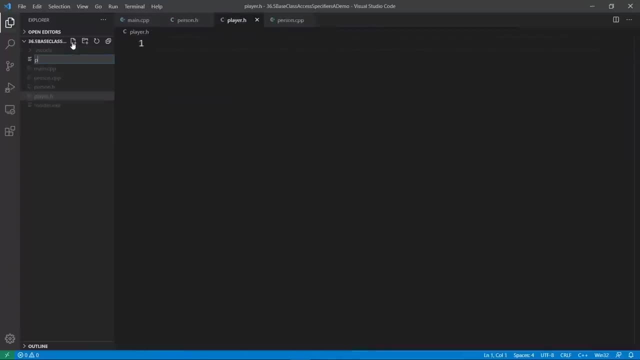 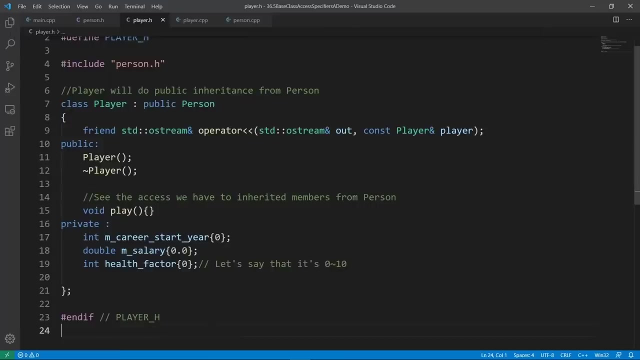 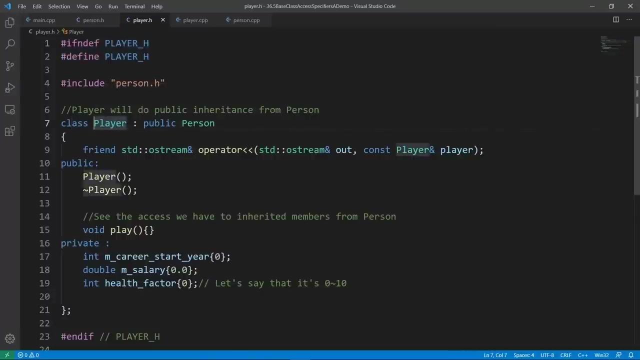 and we're going to say playerh, we're going to put in a cpp file, we are going to hop over in the header of player and put in our class. let's close the left sidebar here so that you can really see everything. we have an include guard in. we have the class player declared it is going to do public. 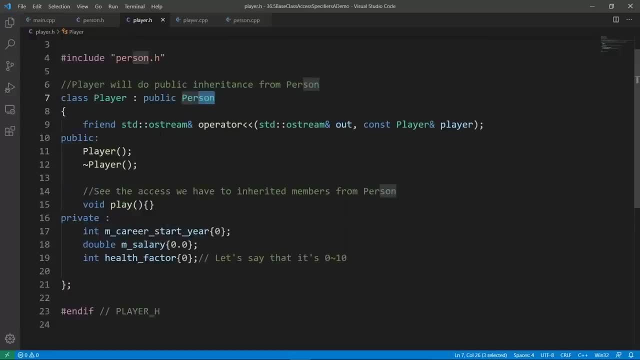 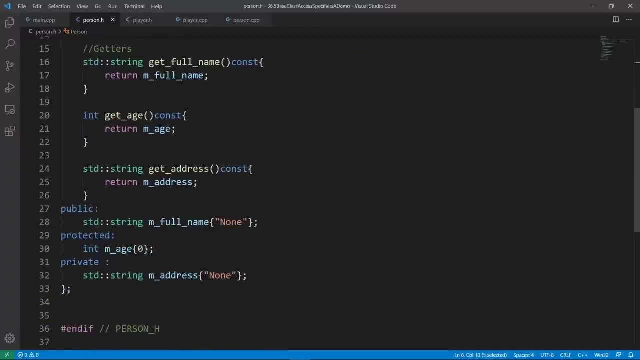 inheritance from person, and what this is going to do is that anything that is public in person is going to stay public in player, anything that is protected is going to stay protected in player and anything that is private is going to stay private. so we want to be able to access private data from a person object. for example, we can't access the. 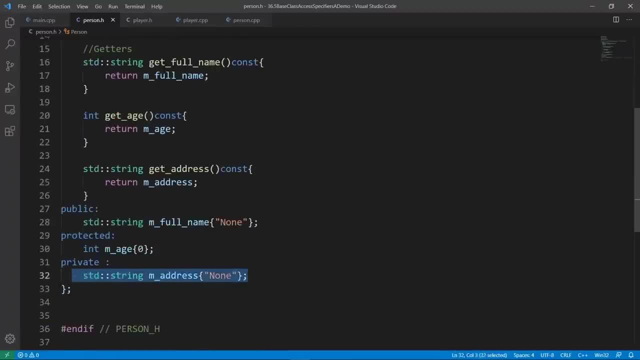 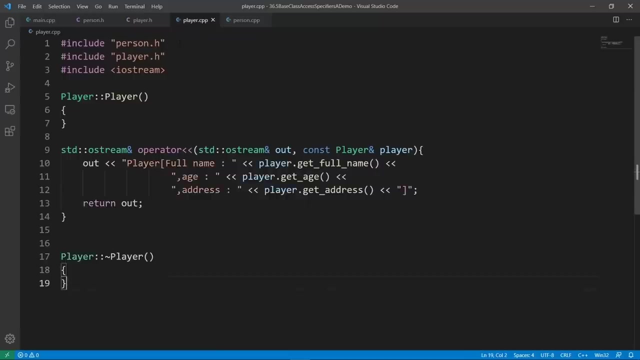 address member variable here because it is private, but we can use the full name and the age from the derived class. sure, we have a cpp file and before we try things out, so let's hop over to the cpp file and put in a possible implementation. we are going to include the person and player because we're going to be 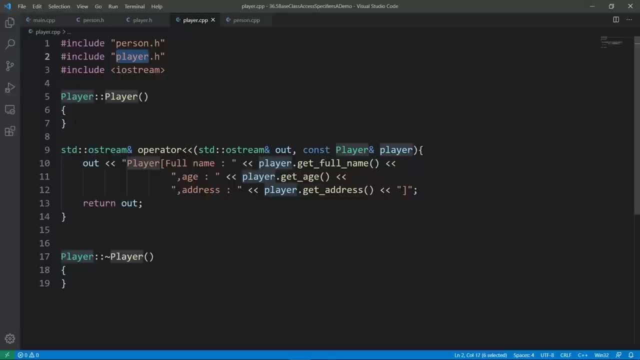 using these and we are going to set up a constructor which is not going to do anything for a player. we also have our output stream operator, which is going to print the data. it is going to be using the getters we have in the base class and we have 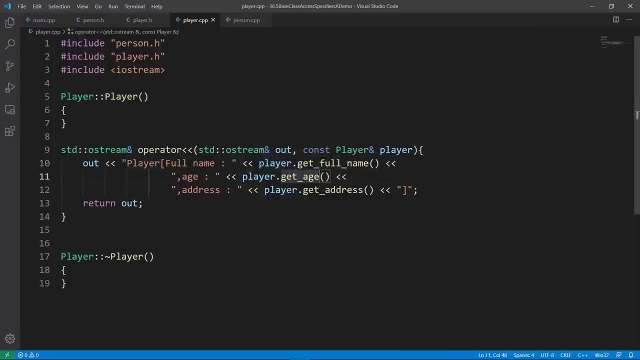 access to them because we are doing public inheritance, so they are going to be public and we can call them from the outside like we are doing here. notice that this is an outside player object and we are calling our public members on that and this is going to work. we. 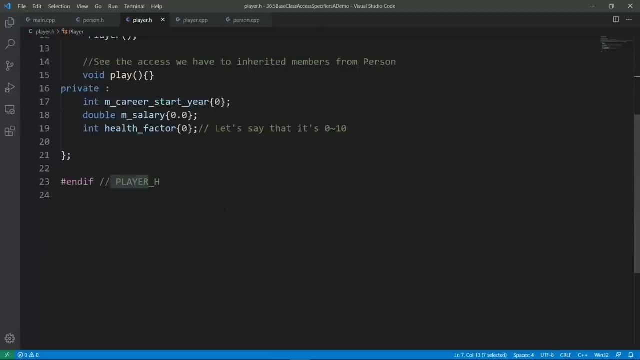 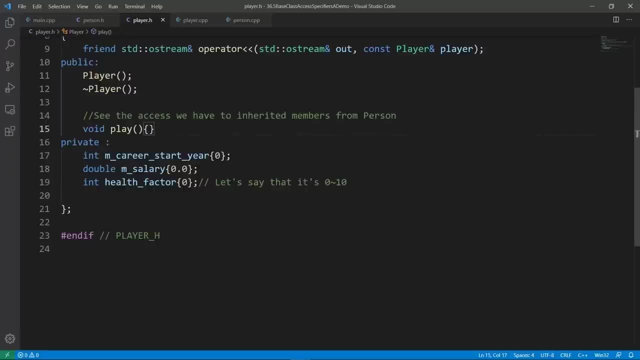 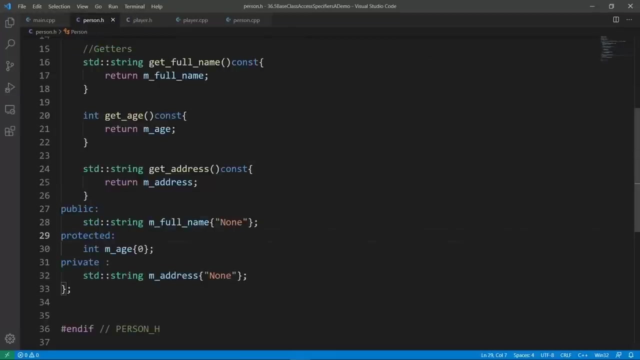 also have a destructor and which is really not going to do anything, but we're going to keep it in here because it's not going to hurt. so now what we want to try out is to see if we can access fans from the base class. the first thing we have in the base class is the full name, and i think we can. 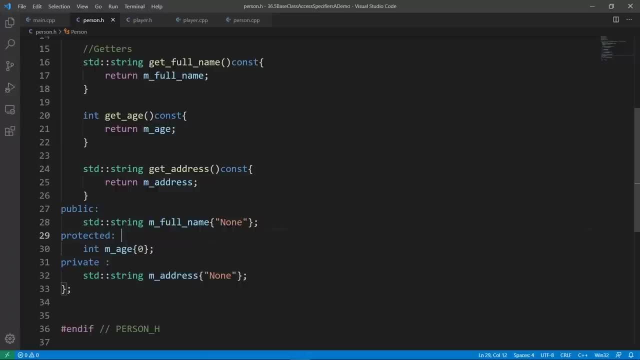 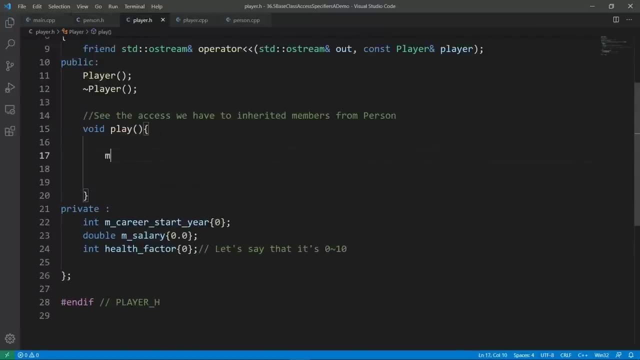 actually copy these things or we cannot just use them: m full name, m age and m address. we're going to try and use them in the derived class. so let's try and say m full name and change the full name, for example, to be daniel gray or john snow, and we're going to change the age to be 55- why not? 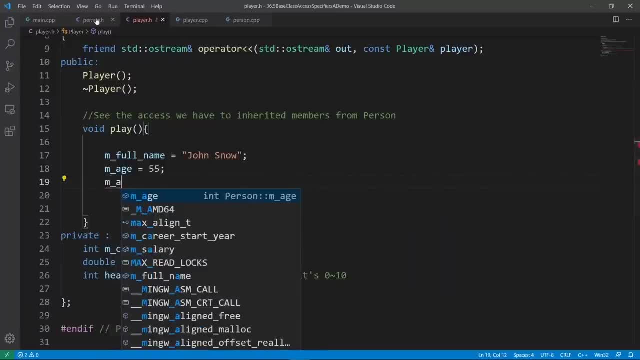 to try and access the address. let's see what we called our address member variable. it is m address. we can grab that and use that in our class. if we're trying to access that, we're going to get a compiler error because that's going to be private to the base class. you notice that if we even try. 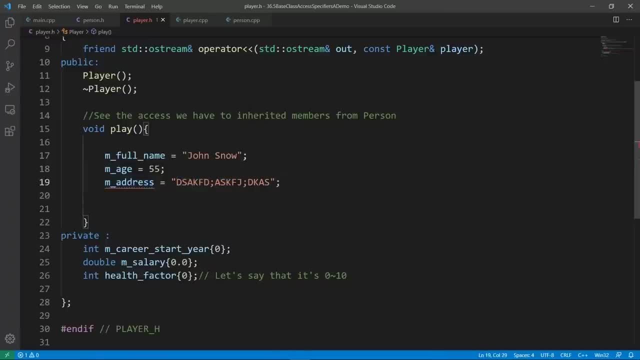 to put some junk data. we're going to have a squiggly line because this is not accessible here and visual studio code is going to say that this is not accessible because it is private to the base class. so we can access m full name because it was inherited as public. so this is going to be. 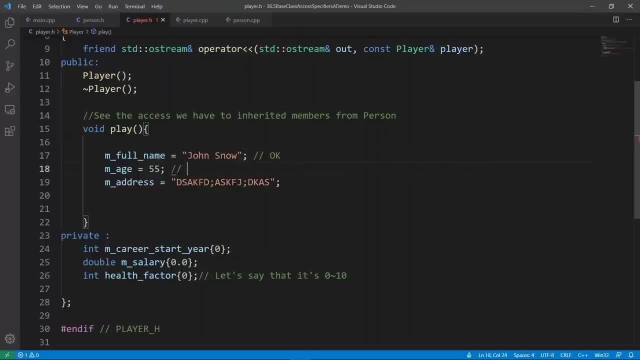 okay, we can use age, because it was inherited as protected. we can use it in a derived class. but we can't use the address because it was inherited as private and it is private to the base class. so this is not going to work. even if we try to compile our code, we're going to get a compiler error. let's try to do that. 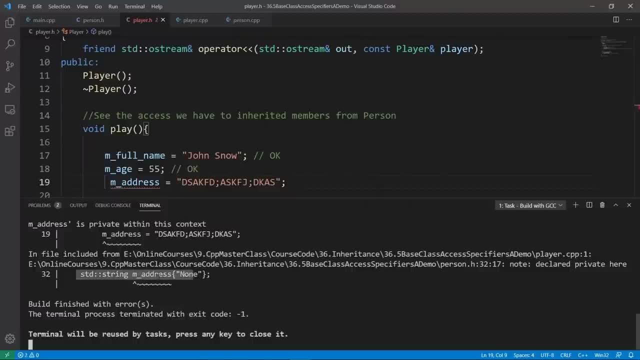 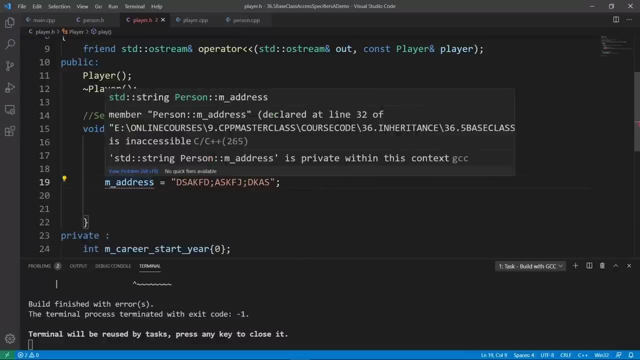 so that you can really see for yourself. okay, so we have a compiler error and this was declared in the base class as private. this is what the compiler error is saying, so we shouldn't really be doing this. the derived class has no business modifying a private member of the base class. this. 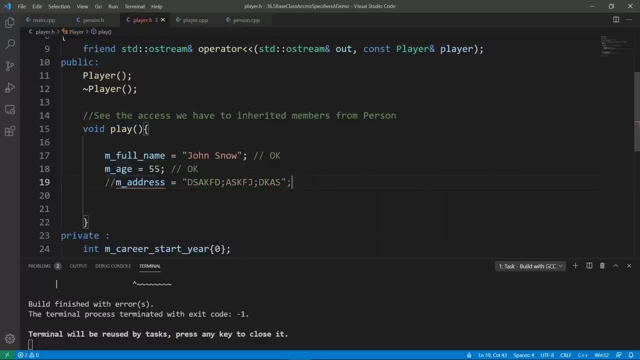 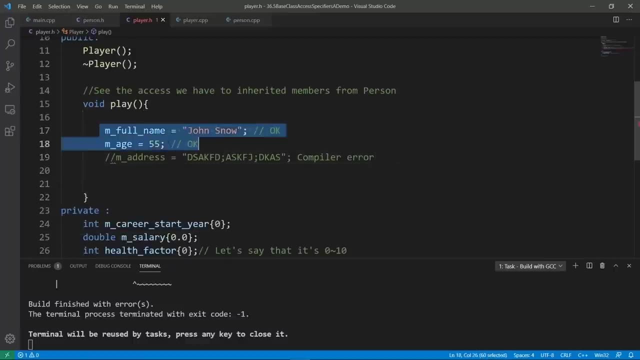 is the message here. so we're going to comment this out and say that this is going to give you a computer, but we are also going to create a player object and try to access these guys and see how access is from the outside. so we're going to go in the main cpp file and we're going to include 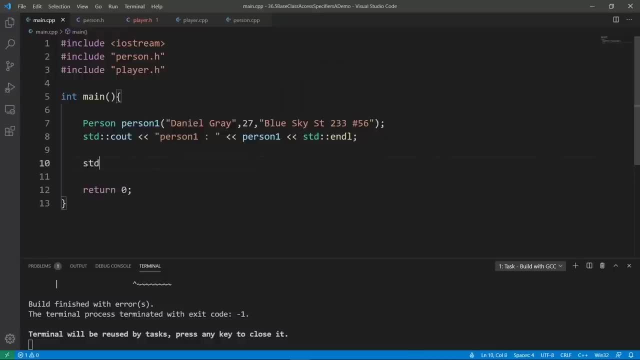 player dot h and we're going to create a player object. we can put in a separator and say a bunch of dashes here. this is going to do. i think this is going to work and we're going to create a player object. we can say player and player and not put any parentheses. 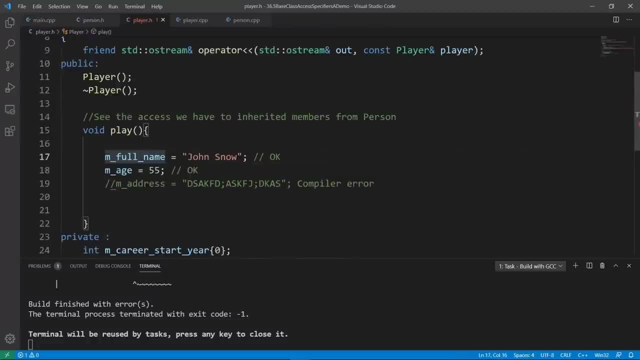 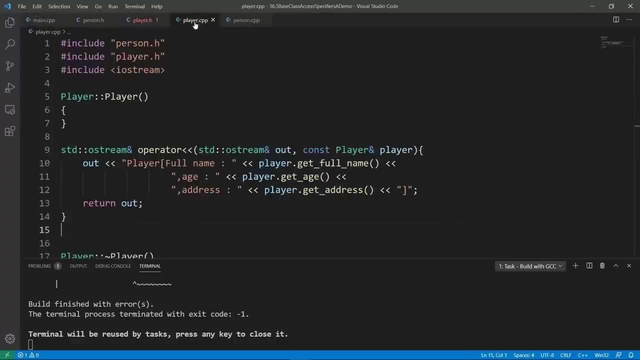 here. this is going to call the default constructor that we have in our player class and we can try to use this. but before we do, let's try and build and see that this is going to world. just fine, we're going to build with gcc, let's do that. we're going to see that the world is. 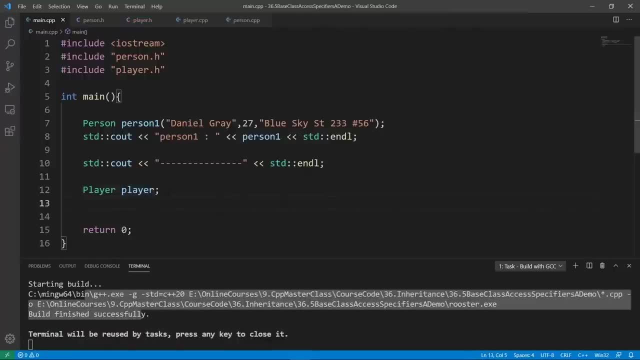 good, we can try and access stuff from this player object. we can say player and say m- full name. you see that this is accessible. we can actually change this to samuel jackson. we can do that. but if we try and say player m h, we're going to see that this is not accessible. 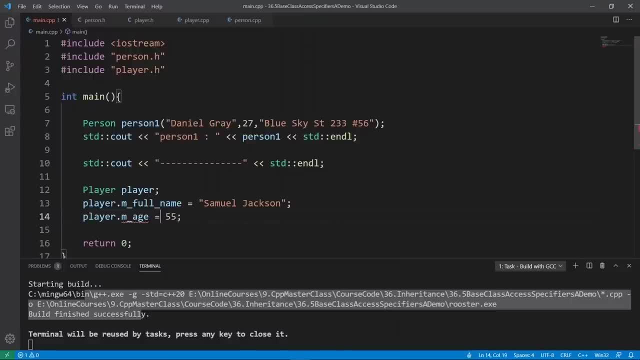 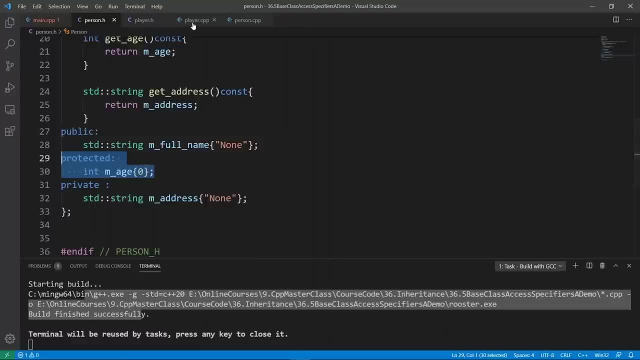 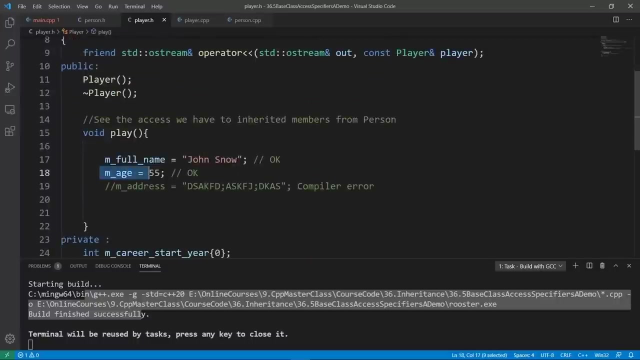 here because this was inherited as protected. if we go back to person, we're going to see that the age is protected so it will be accessible in derived classes, just like we did in our play method of the player class. but we can't access the age from the outside of a player object because that's 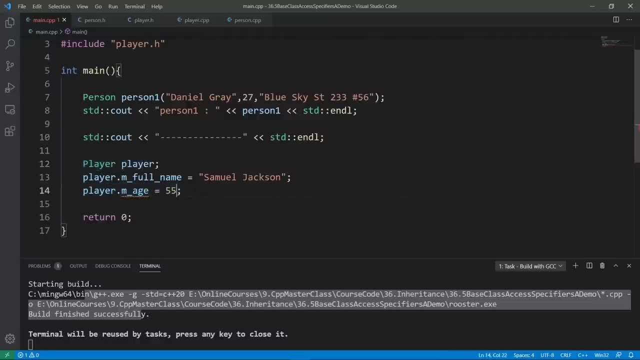 not going to be accessible from the outside of the player object, so we're going to do that from the outside. this is a defining feature of the protected access level. so this is not going to work. even if we try to build, we're going to get a compiler error along the lines of: this is not. 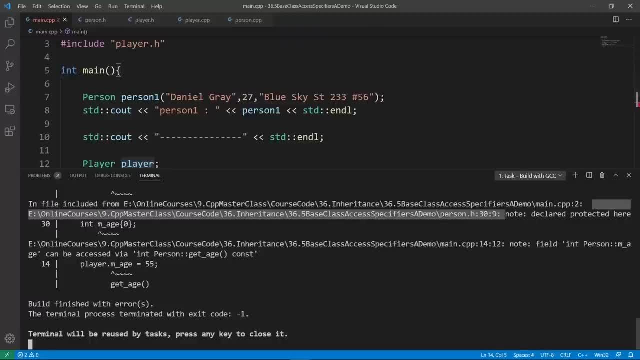 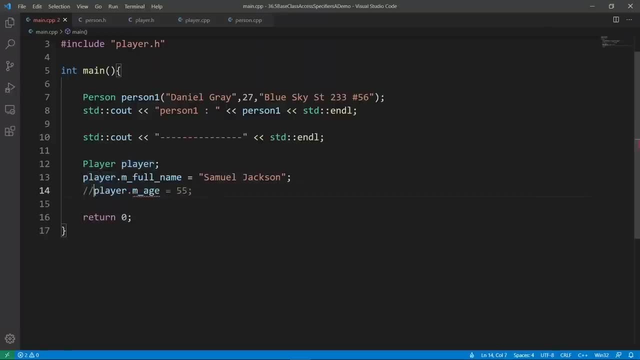 accessible in this context and it was declared in the base class, so we can't really access it from the outside. this is the compiler error here, so we're going to comment this out and say that this is going to give you a compiler error. okay, so i hope you know that you can't even have a chance. 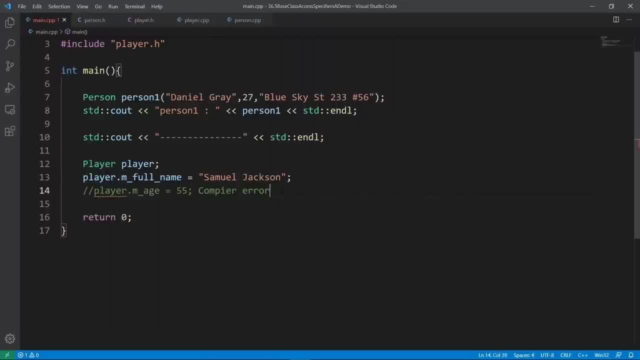 to access it from the outside. you can't even access it from a derived class. so if we try and do a private member of a base class from a derived object in the main function, like we do here, so if we try and do player and say m address, this is not going to work okay. so if we try to change this for 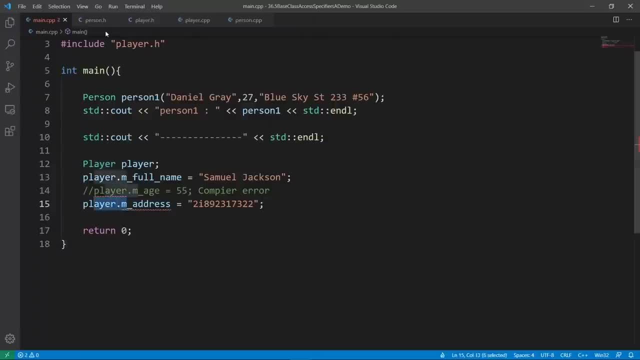 example, to some junk data. this is not going to work. we're going to get a compiler error because this was declared private in the base class and it is private to the base class. you can't really access it from the outside, let alone access this on the outside in the main function. so this is not going to work. it is going. 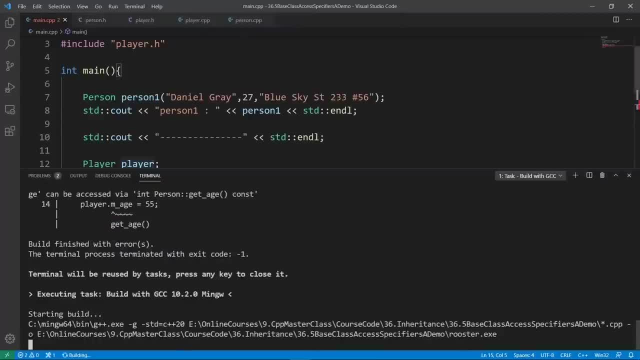 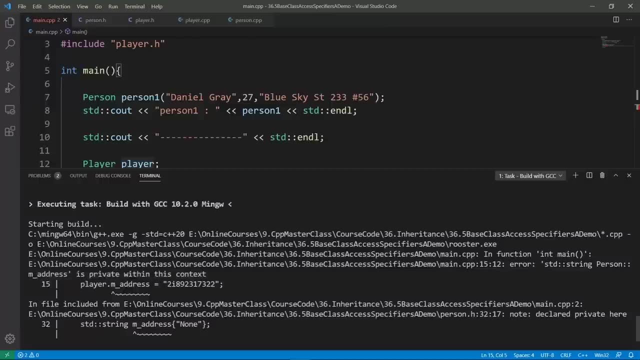 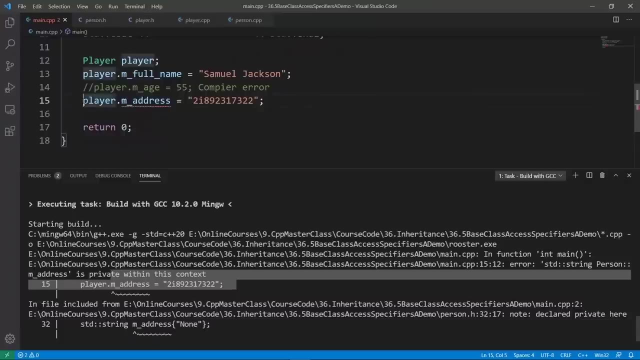 to give you a compiler error, but we're going to weld and show you the compiler error because we are learning here. so we're going to get a compiler error that says m address is private within the context where we are trying to use it, so we can't really use it from the outside. here again, this is. 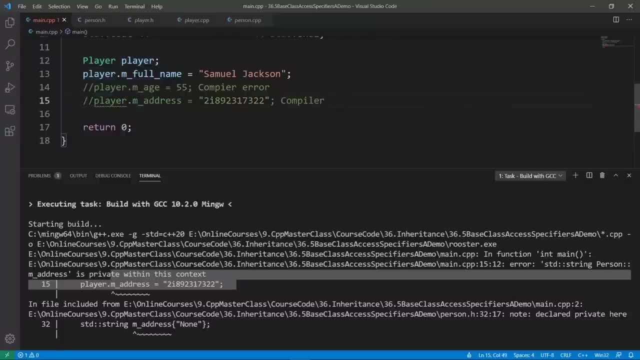 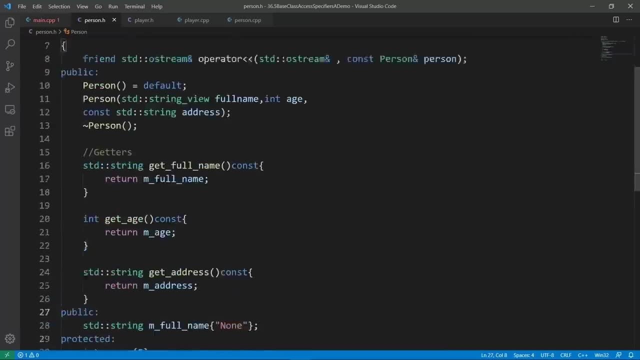 going to give us a compiler error. let's say that here, and this is really what i wanted you to learn really well with this interface, but you wouldn't be able to fix the quê wurde where x- i'm not gonna prove that this is going to be valid- and x is either as an order or in order element, as showing. 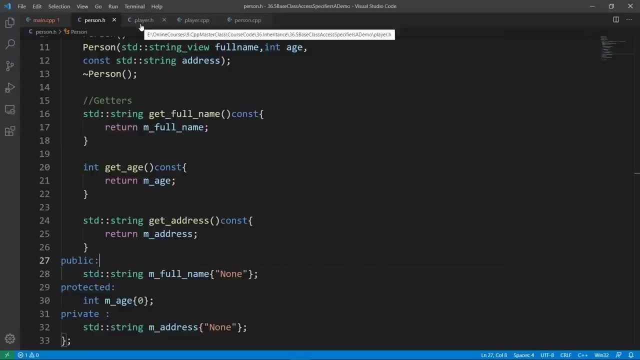 you that it will be valid a month later. click on yes, then it will completely change the curly circle. and then, when you download a new application and talk to them about public, andarez, but before that go, select your anything that is safe to access from a base. and next talked about public. 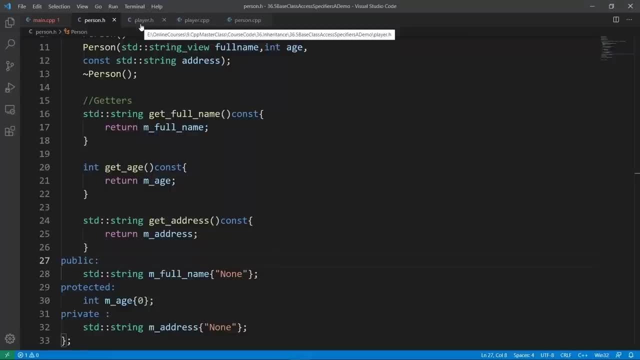 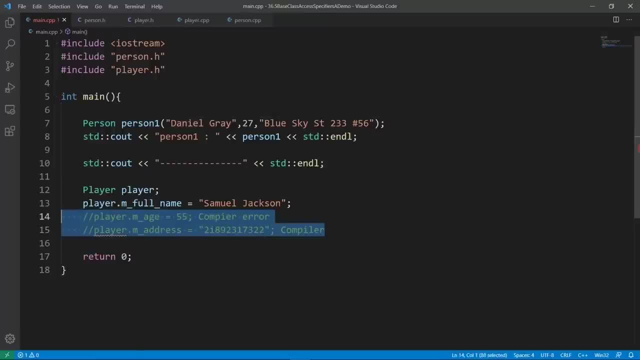 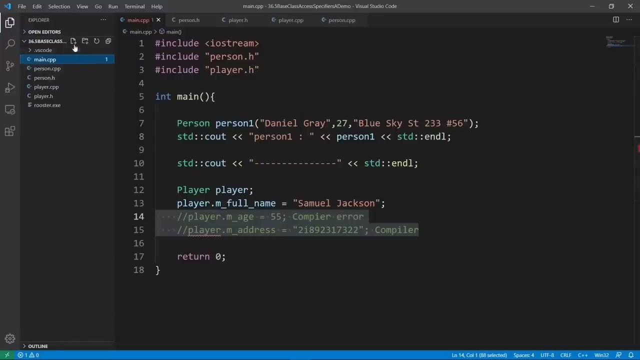 inheritance. anything that is public in the base class is going to be public in the derived class. anything that is protected is going to stay protected, and what that? now that we have this in place, we're going to set up another class that is going to do protected inheritance and that's going to be our nurse class. so we're going to put this in. let's. 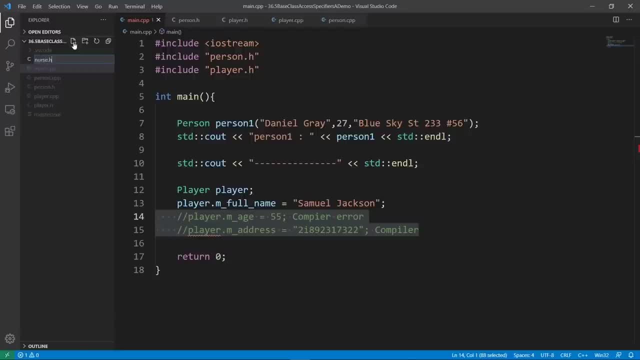 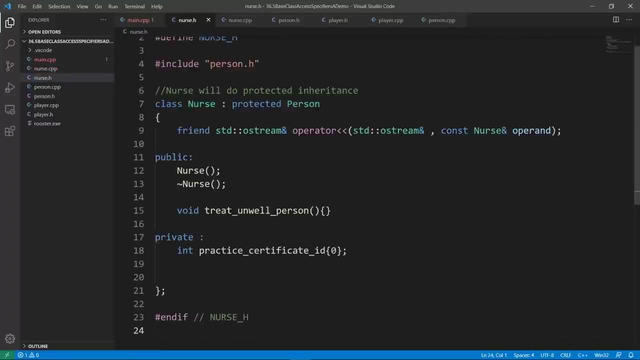 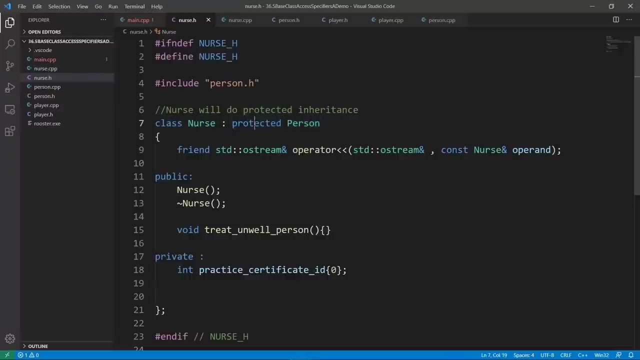 put in a nurse header file. this is going to be nurseh. we're also going to put in nursecpp, okay, so we're going to head over in the header file and put in the code for our nurse class. we're going to say class nurse and say protected, to mean that we want to do protected inheritance. 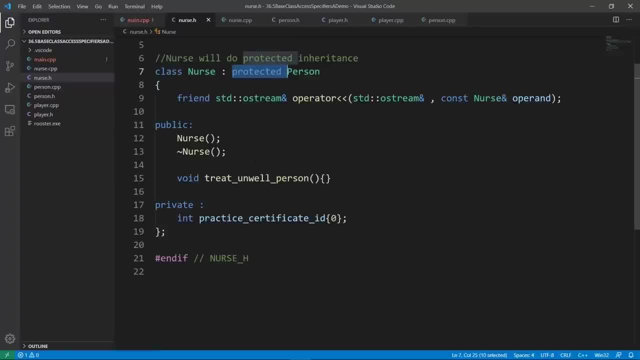 and what this is going to do. anything that is public in the base class is going to be protected in the derived class, which is our nurse class. anything that is protected is going to stay protected. anything that is private is going to stay private to the base class. this is what we 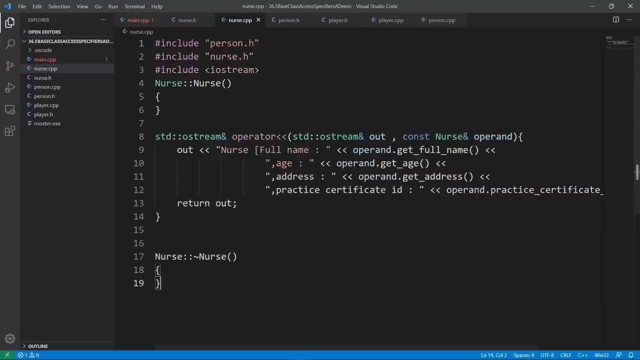 mean here: okay, now that we have this and we can put in the implementation for our nurse class and we're going to have the constructor and we're going to have our output stream operator and we're going to have a description which is really not going to do anything because we don't have any dynamic memory allocation in. 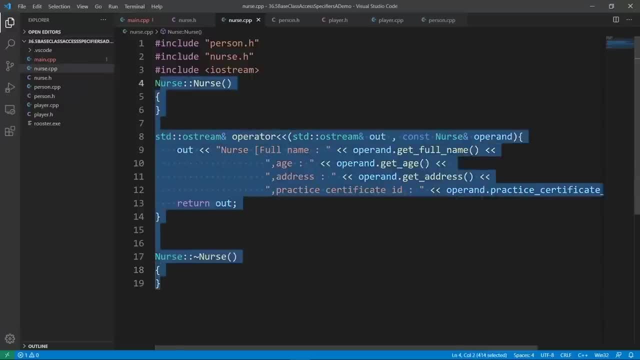 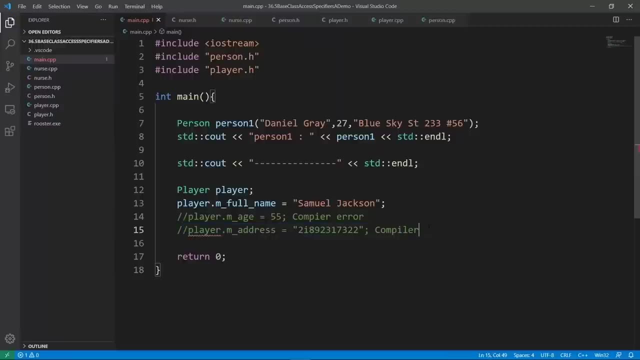 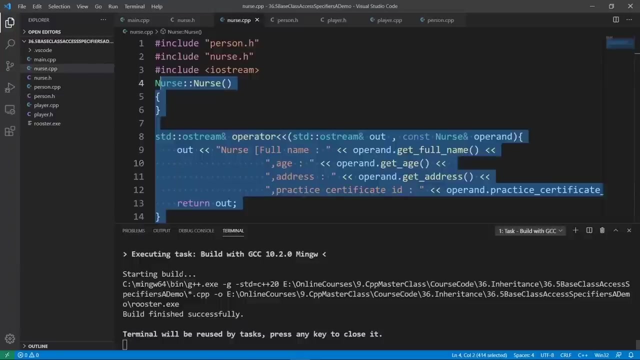 our class. we are going to try and build this code to see that it is going to work. we have a squiggly line in the main cpp file, but it was because of the line 15 here and it has been commented out. let's see if we can build this program. okay, you see that the world is going to be good and we are. 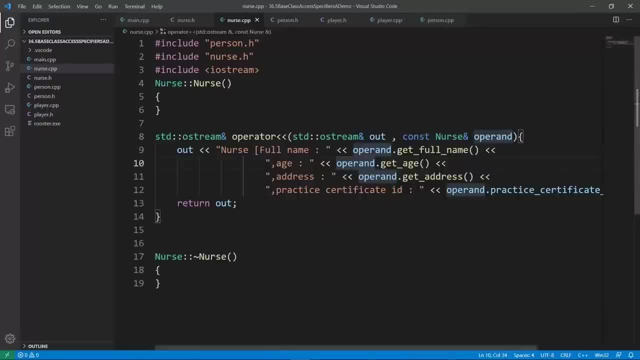 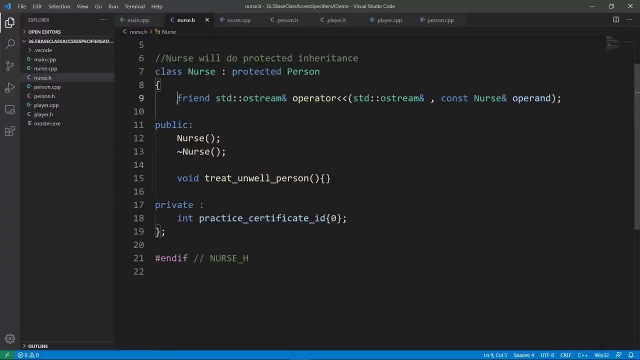 able to call flanks from our output stream operator. you see, we have a nurse operand. we are able to call this get full name and get age member function because they are now protected in the nurse class. but we are able to call them from the outside because this operator is a friend of our nurse class here. i want you to 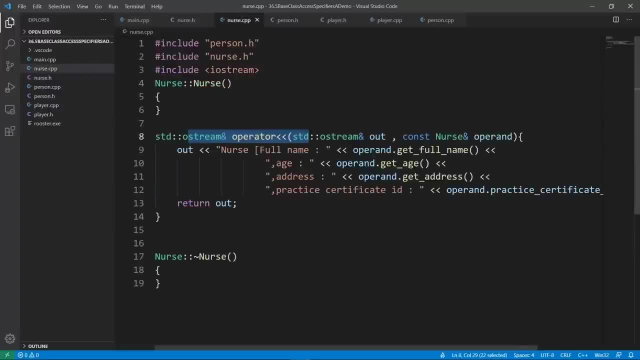 say this, some of you are going to ask: aren't we using an object and calling a method using the dot operator? this qualifies as calling thanks from the outside, and, yes, that's true, but this method is really like a member function in that it has access to private and protected data from our nurse class and the 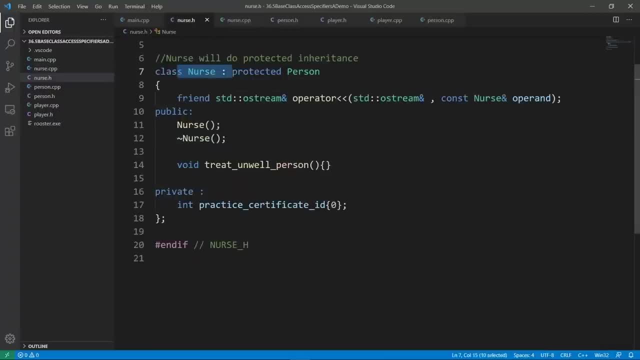 reason is it is a friend of the nurse class here. that's why we are able to do something like this. but what i really want you to see, now that that doubt is cleared, is the kind of access we have to things from the base class. we will still be able to use m full name here, because it was inherited. 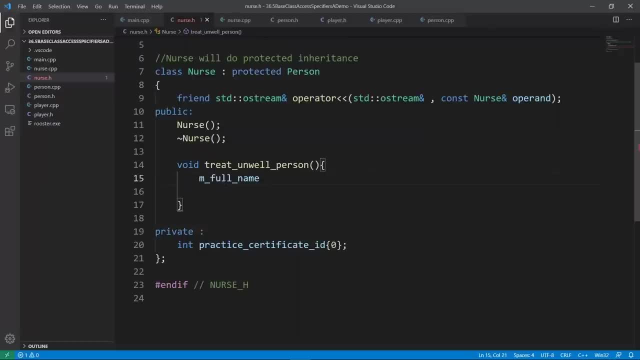 as protected, so we can use it from a derived class. we can say m full name john snow. this is going to work because this was inherited as protected. now it is protected in the eyes of the nurse class. this is what we mean here. so this is okay, this is going to work. we can get the age. we can use that. 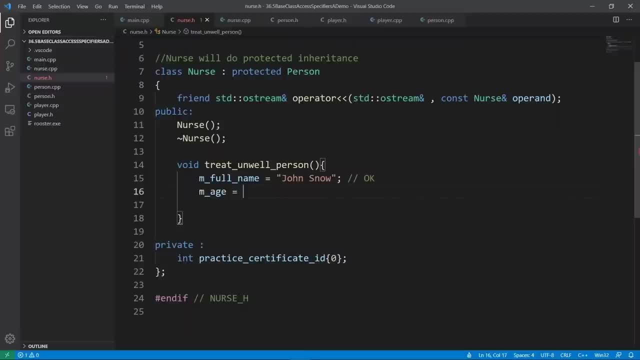 and we can say john's and we can say 23, for example. this is going to work because this is protected, but we can't use the address. if we do that, we want to be able to change it- we will get a compiler error because this is private to the base class. this is the same thing we saw in the 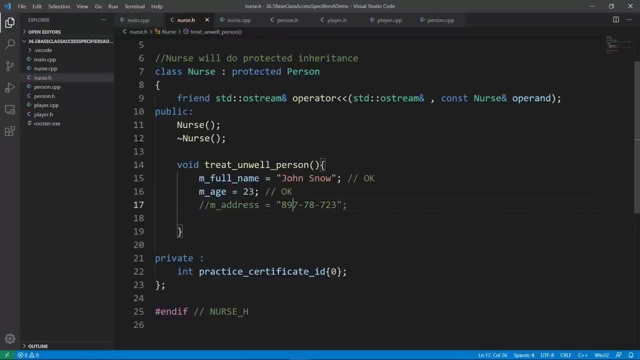 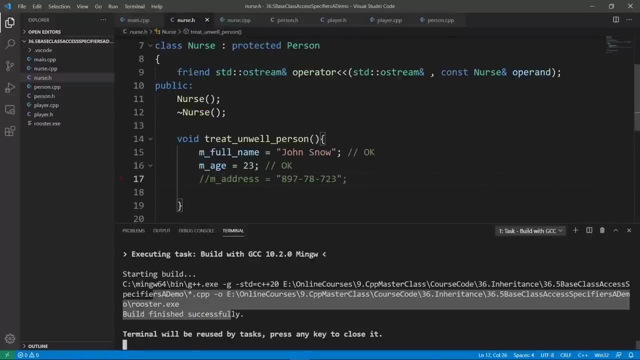 last lecture. this is going to give us a compiler error. if we try to build this program, let's try and build it to really prove this. the world is going to be good without line 17 in here. but if we uncomment it and try to build the program, let's do that. we are going to get a. 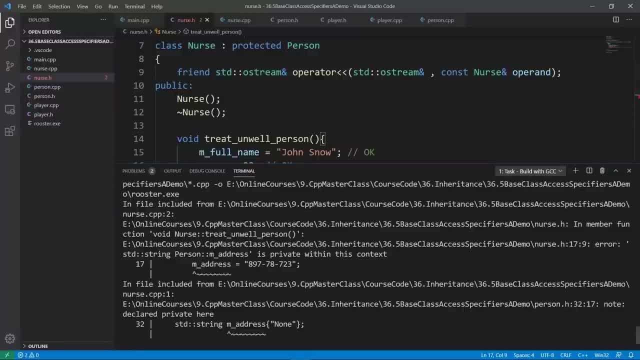 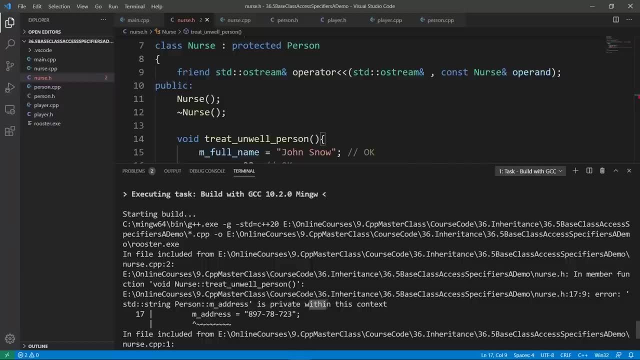 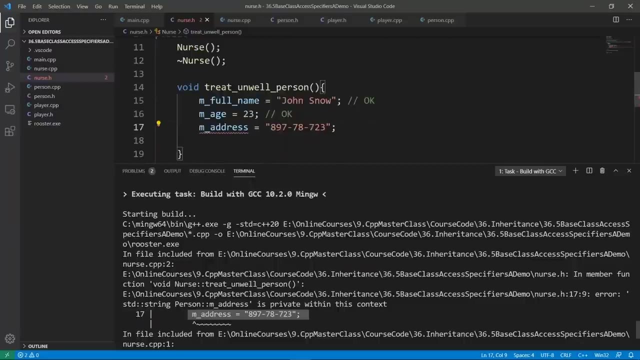 compiler error. and the compiler error is going to say: let's go up and see if we can get this message. it's going to say m address is private within this context where we are trying to use it and that's line 17 of the nurse class. if we go there, we're going to find the offended line here. 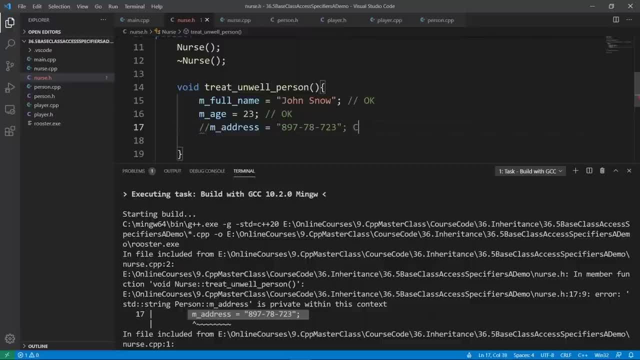 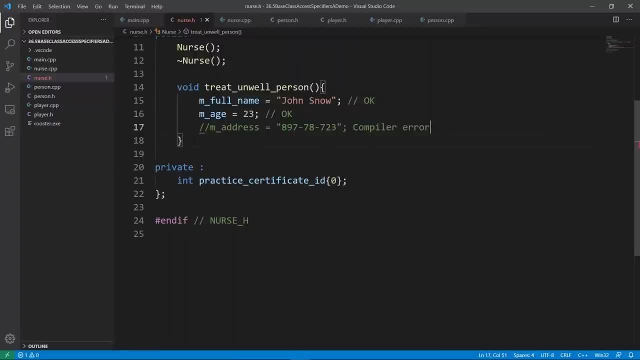 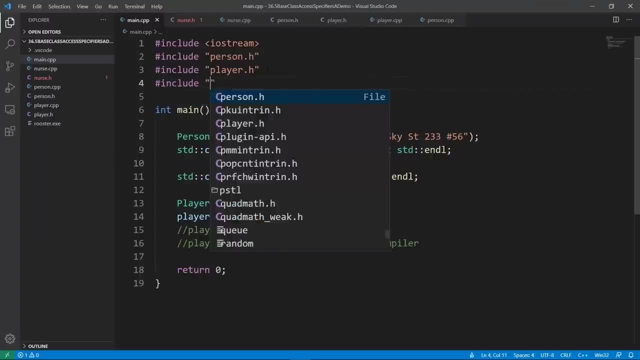 so we're going to comment this out and say that this is going to give us a compiler error. okay, so you shouldn't do this. now that we know things from the inside, let's see how things fare on the outside. we are going to hop over to the main cpp file and include our nurse class. 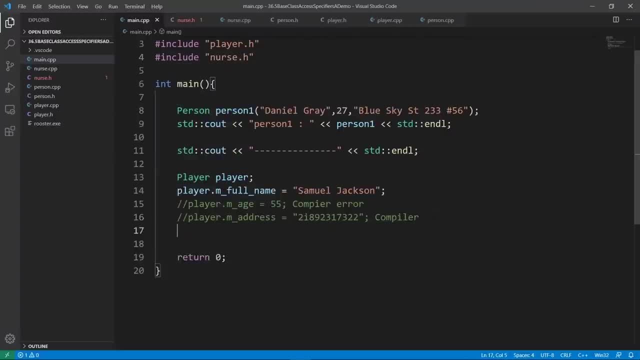 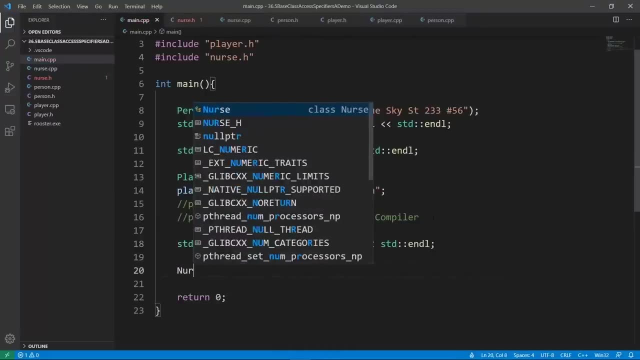 and we're going to create a nurse object. we can go down and say, stdc out and we're going to put in our dashes and we're going to create a nurse object. i think we have a default constructor for a nurse. we're going to say nurse1 and we're going to basically 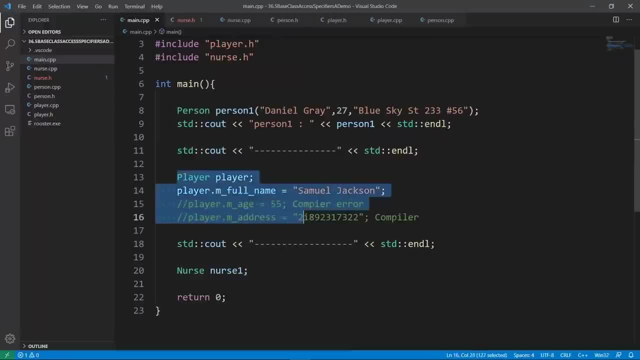 try and do the same things we did for the player object from the outside. if we try to access the full name now, it's not going to be accessible because it was inherited with protected access level. so if we do nurse and say m full name, you're going to see that. 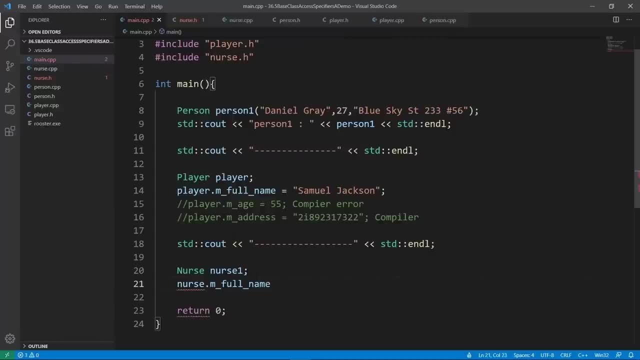 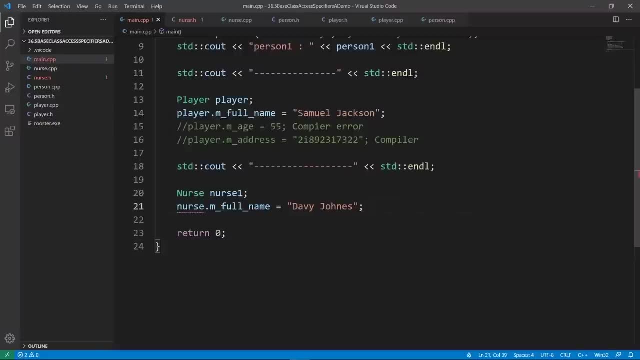 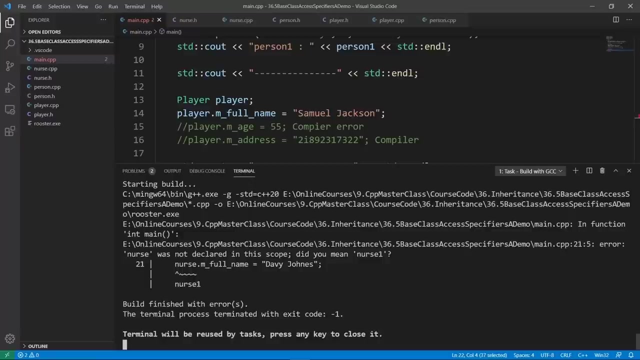 autocomplete is not here. this is a good sign that this is not accessible from this place. if we say davy jones, we're going to get a compiler error, and if we try to build, we're going to get a cryptic compiler error. at least i hope so. let's vote. we're going to see that we world with errors. 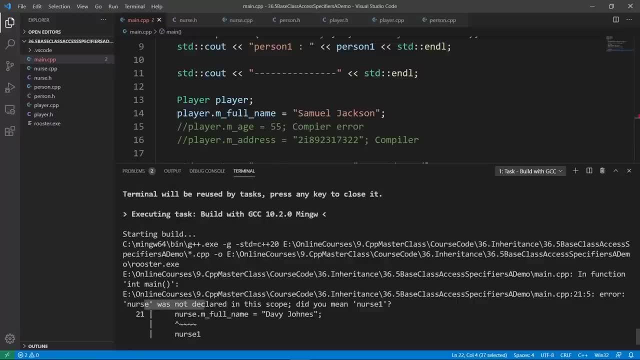 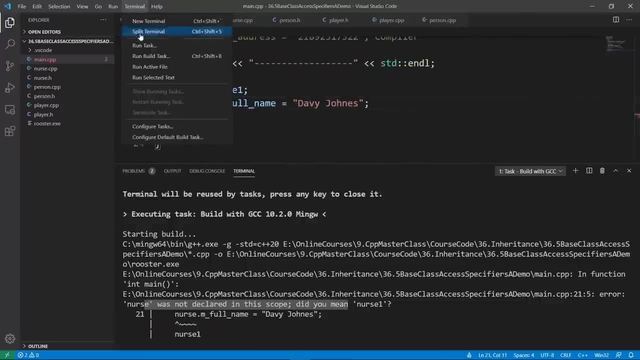 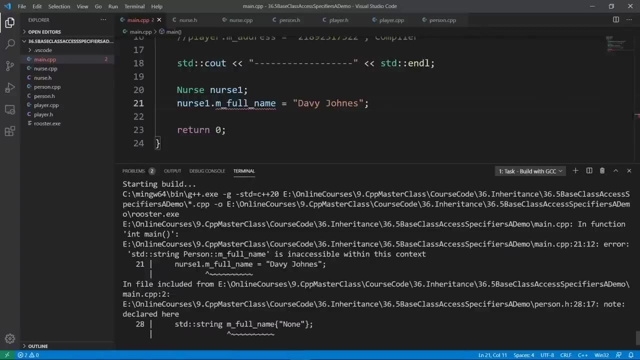 and if we go up, we're going to have our error. nurse was not declared in this scope. did you mean nurse one? yes, we meant nurse one. sorry for that, we're going to build again. thank you, jcc, for pointing this out. we are going to get another kind of error and if we look at our error here, 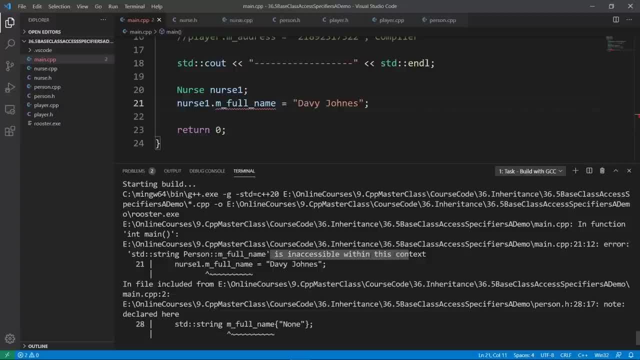 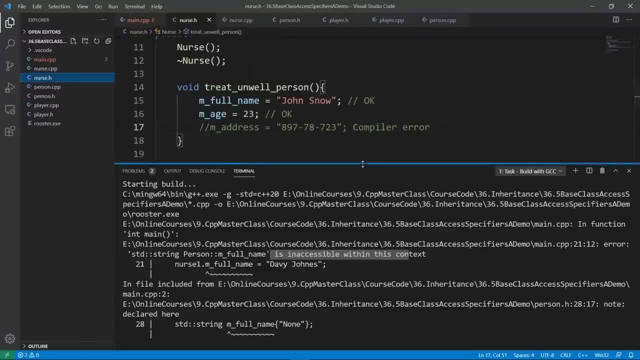 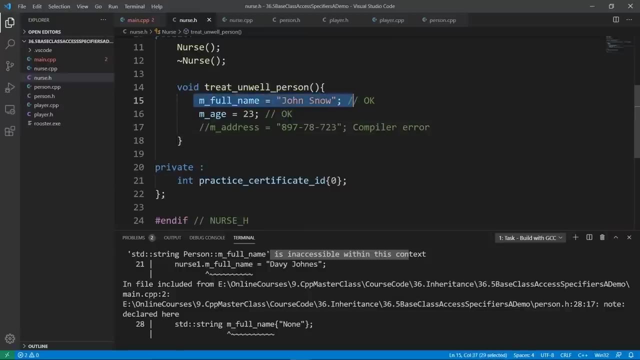 we're going to see that m full name is inaccessible within this context because it is a protected member of the nurse class. now It was inherited as protected and we can't access it from the outside. We can access that from the inside because it is protected, But if we try to 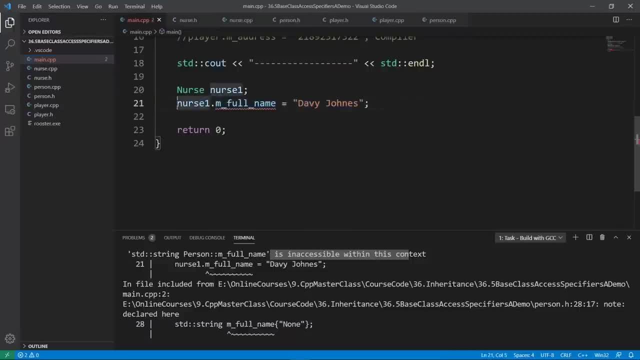 access it from the outside, we're going to get a compiler error, And this is a defining feature of protected inheritance: Even things that were public in the base class are going to become protected in the derived class. So this is the message here and this is going to give us a 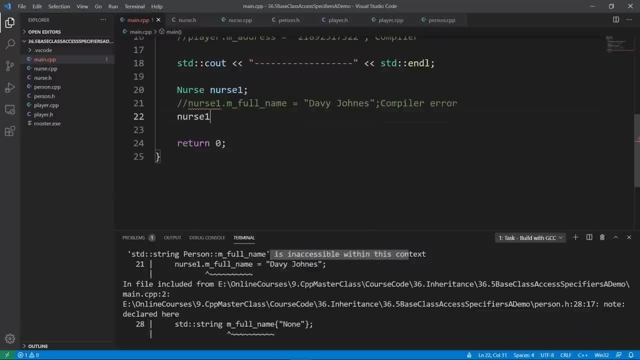 compiler error. Okay, So if we also try to access nurse one and say m age, this is also going to give us a compiler error. Let's try to put in an age here. Let's put in 51.. You're going to see. 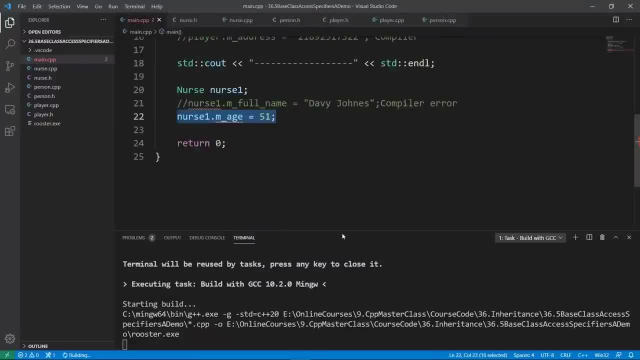 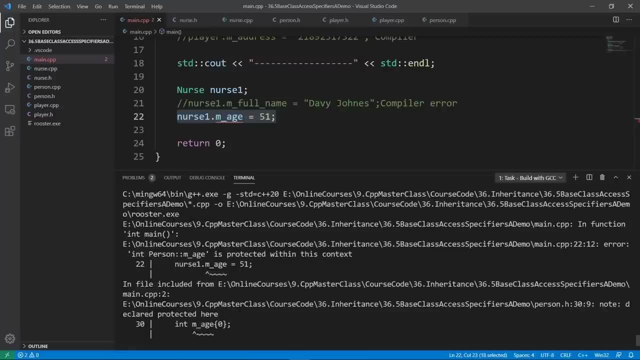 that we're going to get the same kind of error. Let's really try these things out and learn about every possible way we can set up these things. If we look at the error, we're going to see that everything is protected. So if we try to access nurse one and say m age, this is going to give us. 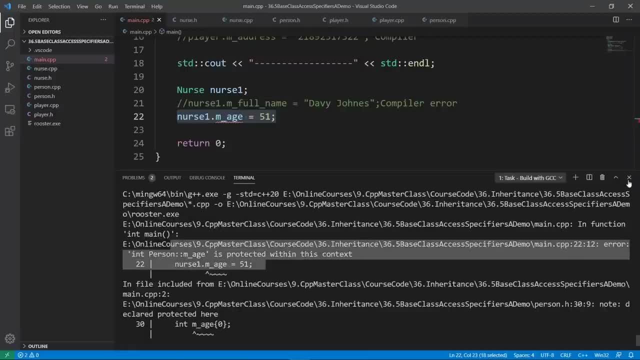 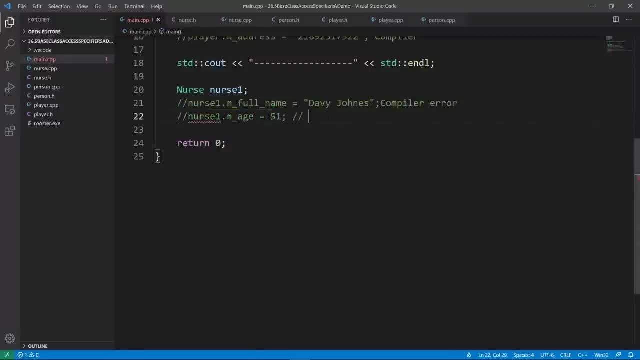 image is protected within this context so we can't really access it. so this is the compiler error we get and i hope you know that if you try and access the address you're also going to get a compiler error because that's private to the base class, so we can't even use that from a derived class like. 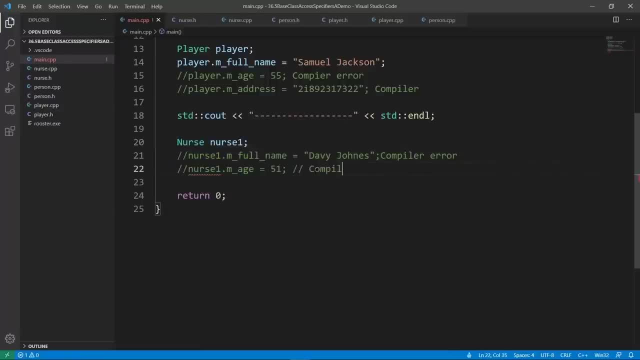 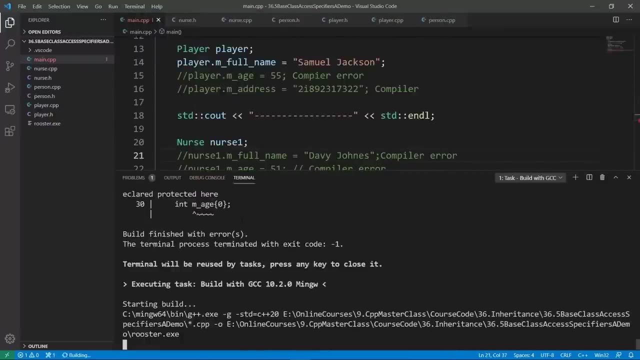 nurse here. that's not going to work. let's say that here we have a compiler error and we're going to set up another class which is going to inherit privately and see how that works out. the class is going to be engineer. we're going to see that the error here goes away, so let's create our 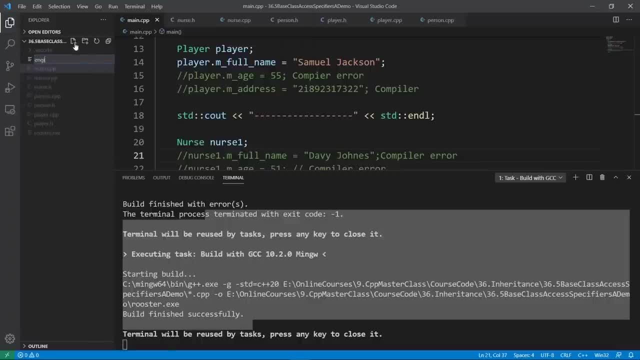 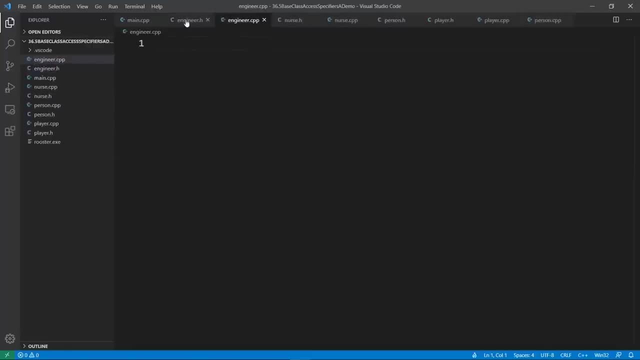 engineer class. we're going to put in a header file that's going to be our engineerh. we are also going to put in engineercpp. okay, so we're going to hop over to our header file and put in our engineer class. we're going to say engineer and say that we want to inherit privately from. 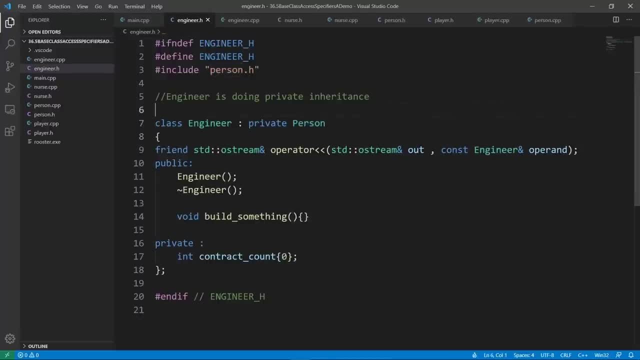 the person class. this is the syntax here and this is going to do private inheritance, and what this means is that anything that is public is going to become private to this class. anything that is protected in the base class is going to become private to this class and anything that was private in the base class is going to stay private we won't have access to. 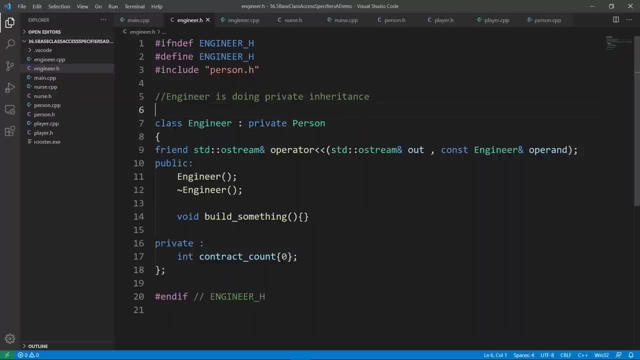 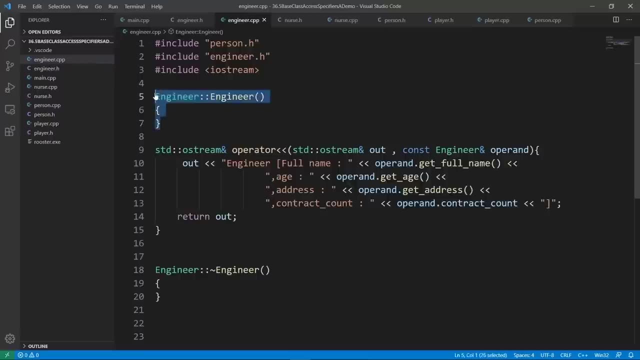 that whatsoever in the derived class directly. we are going to hop over to the cpp file and put in our implementations. we're going to have a default constructor for engineer which is not going to be taking any parameter. we're going to have our output stream operator, which is going to still work because it is a friend of the engineer class. so all these things. 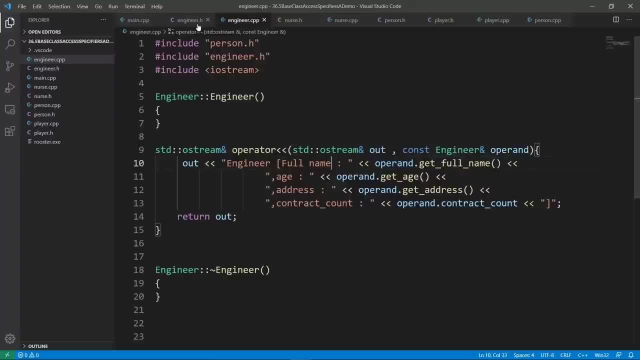 that were inherited to be private are going to be private to the engineer class and any friend of the engineer class will have access to that. that's why we are able to call, get full name, get age and get address here and get these things to work. okay, now that this 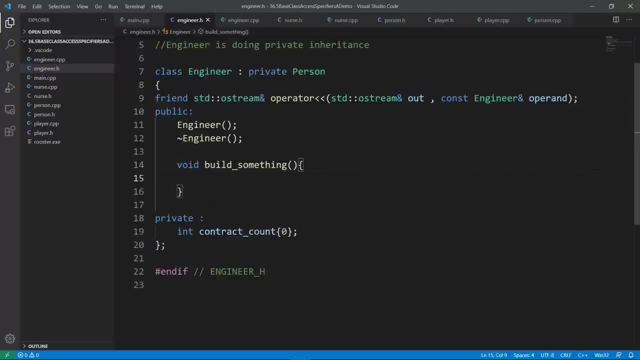 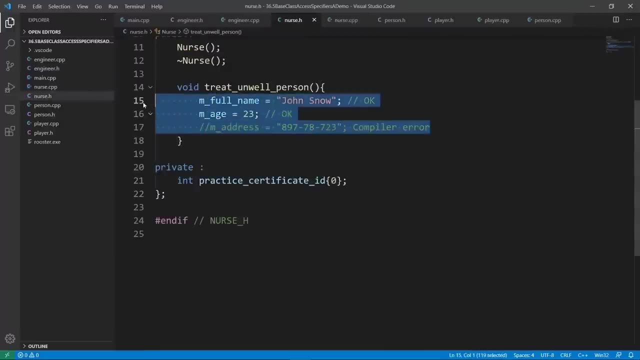 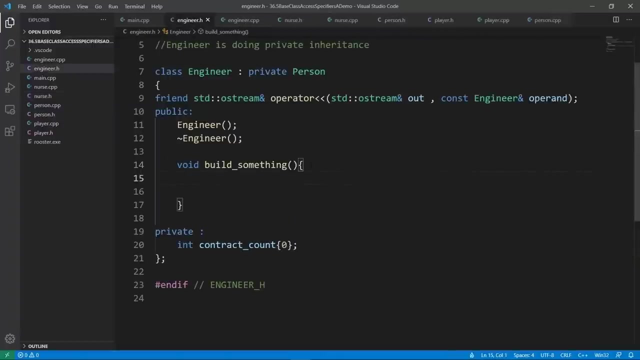 is out of the way we can try and access our thanks. we're going to try and do the same things we did in our nurse header: we're going to copy the code, because we are trying to access the same member variables, and we're going to see how this fares in our engineer class. this is going to save us. 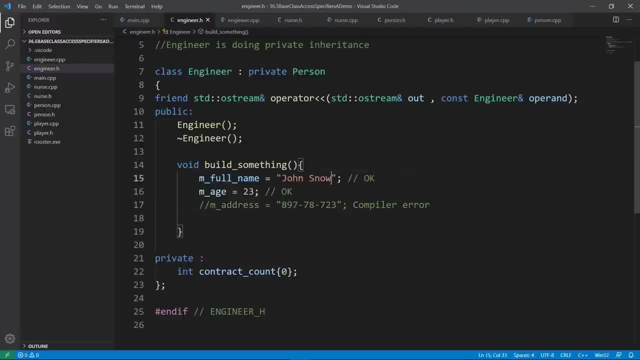 a few seconds. if we try to access the full name, this is going to work because it is private to this class. if we try to access the age, this is going to work because all these guys are now private to this class here. but if we try to access the address, this is going to give us a compiler error. 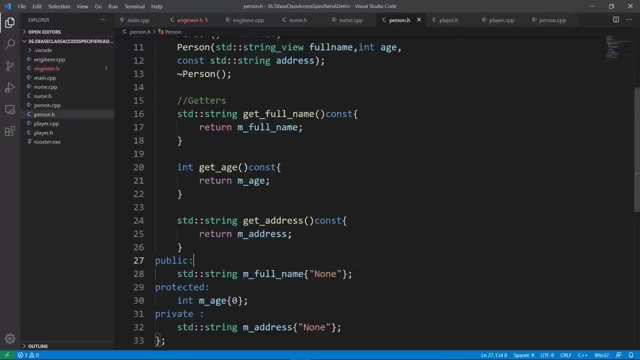 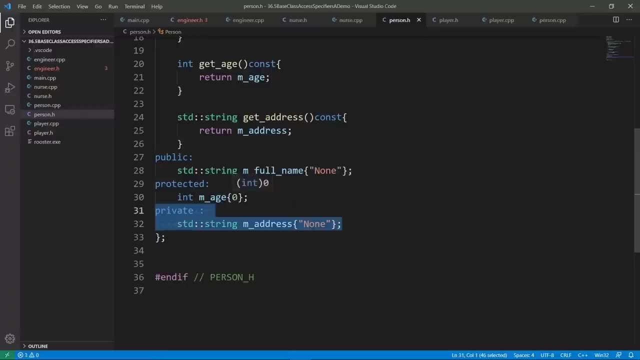 because address is private to the base class. if we go back to person, we're going to see that this is the case and if you try to inherit from this class in any way, you're not going to be able to change this access level. this member variable is always going to stay private to the base class. 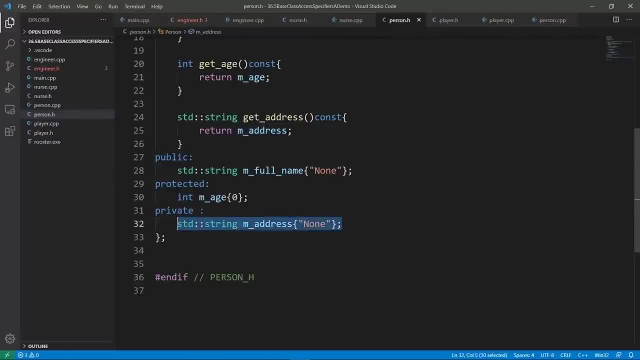 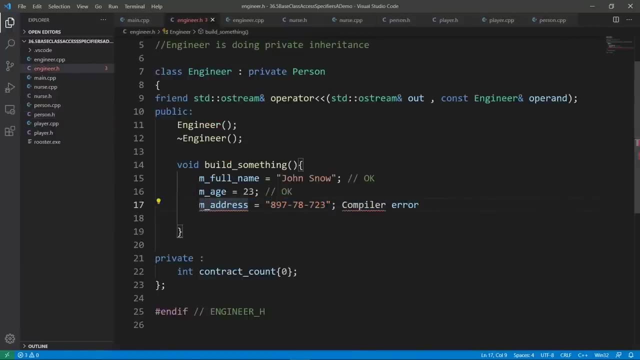 and no derived class will be able to modify or read from this in any way. so this is the setup we have here. if we're trying to build, we're going to get a compiler error. let's first take this out and show you that this is going to build just fine without this line. 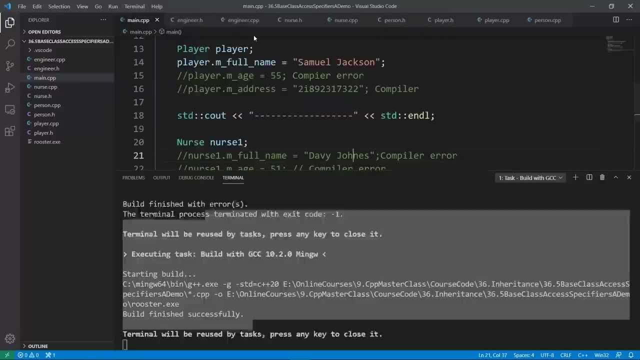 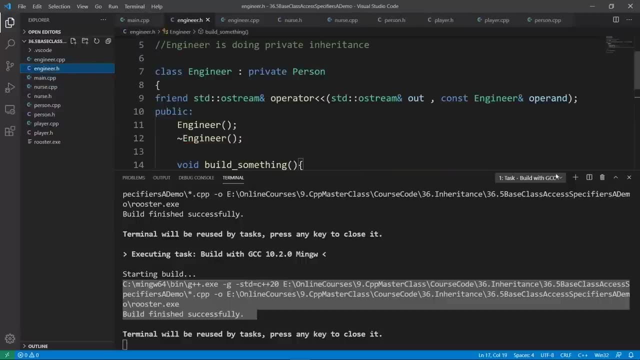 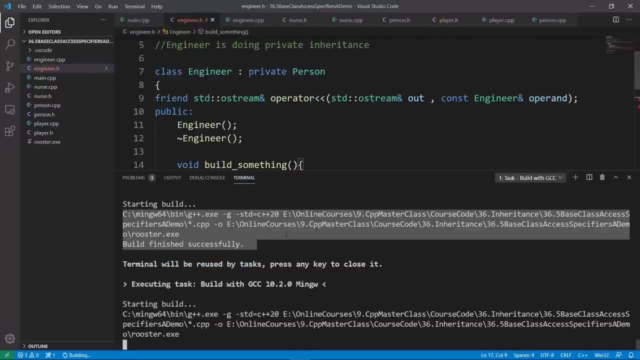 here and i am going to build again and show you that if we bring that in, we're going to get a compiler error. so the both is good. we can go back in our engineer class and bring in the offending line. we can uncomment this and if we're world, we're going to get a compiler error. let's make. 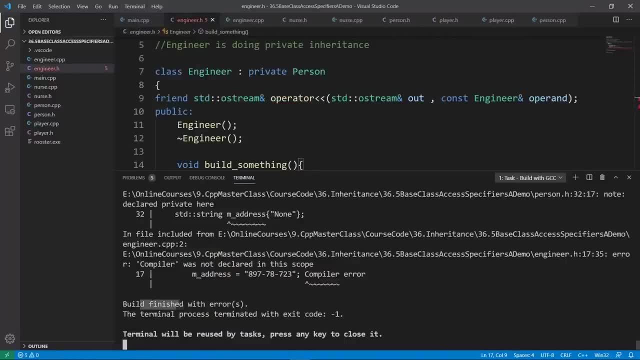 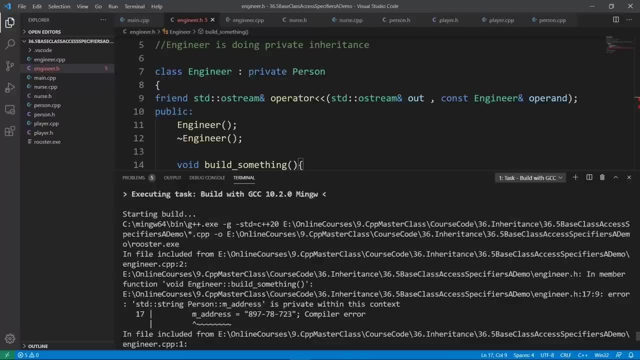 sure you see the compiler error here. so the build was finished with errors and if we go up we're going to see that we have an error here and the error is going to say: m address is private within this context and the context is what we have at line 17 in the engineer class, so we can go there. 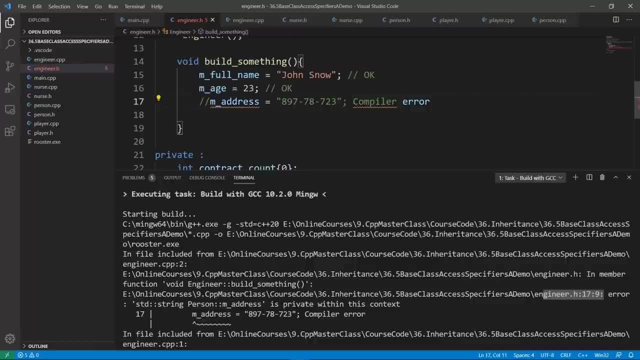 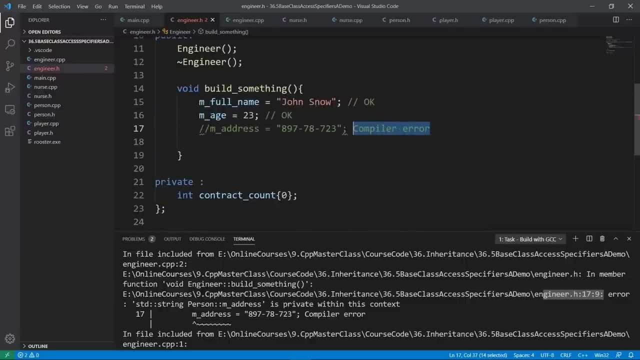 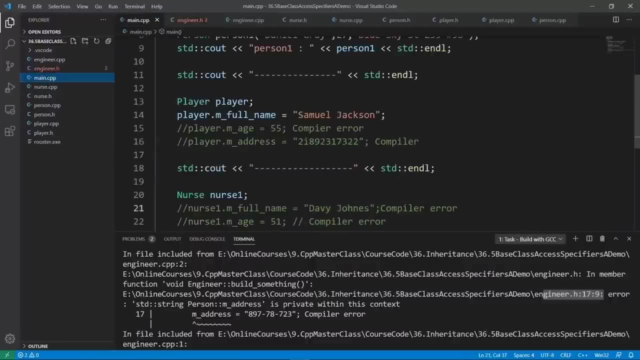 and find the offending line and we're going to comment this out and this is going to give us a compiler error. now you know this. but this is how things are going to work from the inside, but we also need to look at how things fare from the outside. let's go back in our main cpp file. 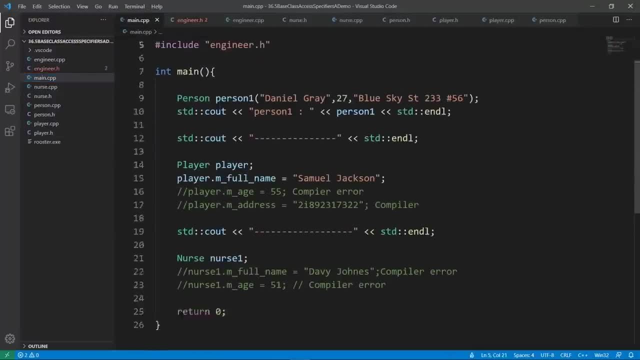 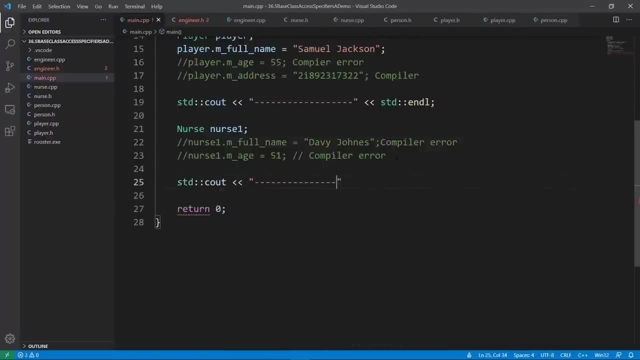 we are going to include our engineer class and we are going to create an engineer object. we can go down and say sddc out and put in a bunch of dashes to separate our things and we can create a engineer object and that's going to be engineer one. 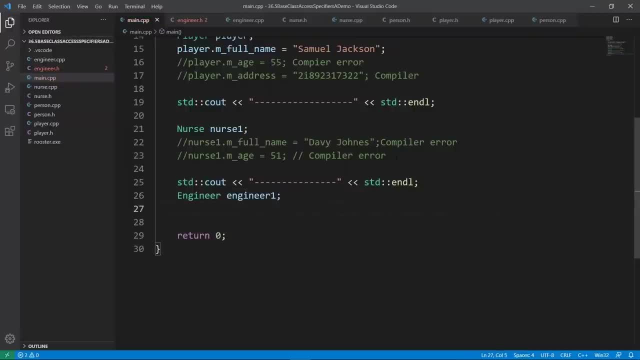 and if we try to access the full name, that's not going to work because it is now private to the engineer class. if we say engineer one and try to say m full name and try to change the name in any way and say, for example, olivier godson- i am making this up, i don't know if this 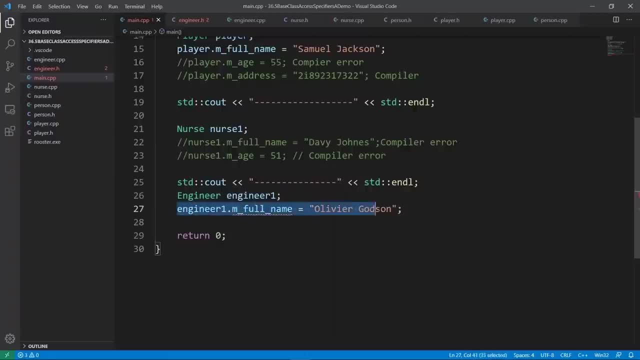 name exists, but the point is that this is not going to work. it is going to give you a compiler error because m full name is now private to the engineer class. it was inherited to be private to the engineer class and if you try to do this, you're going to get a compiler error. let's try. 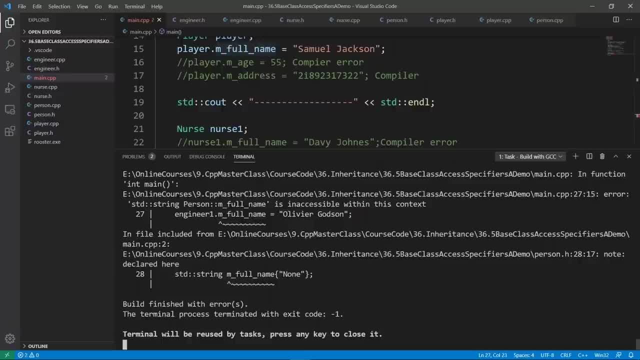 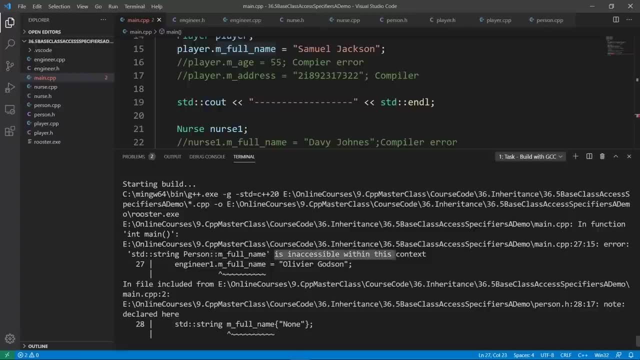 and world with gcc to really show you this. and the world is going to be finished with errors and if we go up, we're going to find our error. full name is inaccessible from within this context and the offending line is at line 27 of the main cpp file. if we go there, we're going to find. 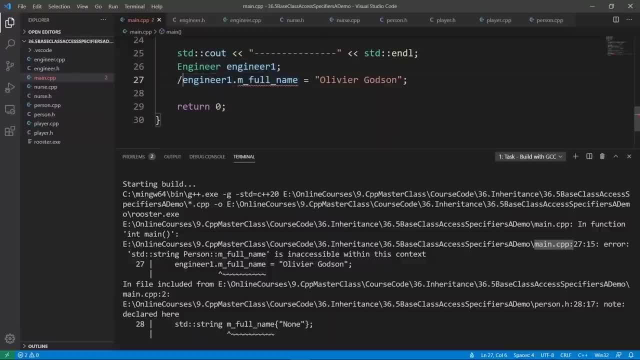 our line and we're going to say that this is going to give us a compiler error. so let's say that we're going to get a compiler error and we're going to say that this is going to give us a compiler error. so let's say that this is going to give us a compiler error and we can't even access. 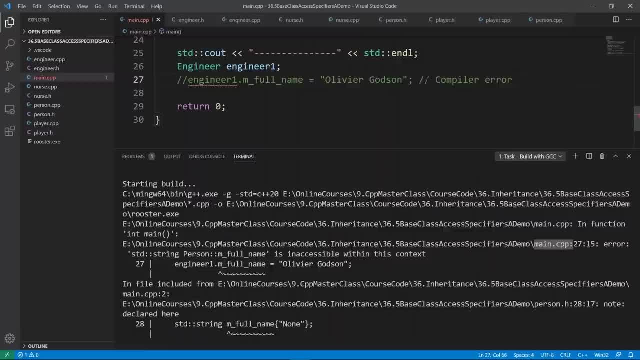 the age and the address member variables. the age is also going to be private to engineer, but the address is private to the base class, so that's not going to work either. so we can't really access that from the outside because it is now private to the engineer class. so let's go down and really 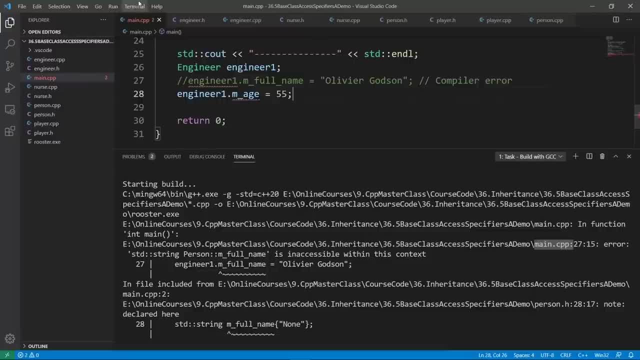 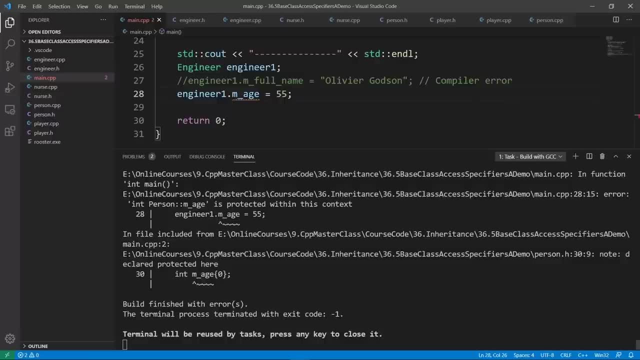 show you that we're going to go down and say engineer one and say, m age, if we try to do that, we're going to get a compiler error. and if we try to build, we're going to get a compiler error along the same lines as what we just got here. the build is going to finish with errors. and if we look at 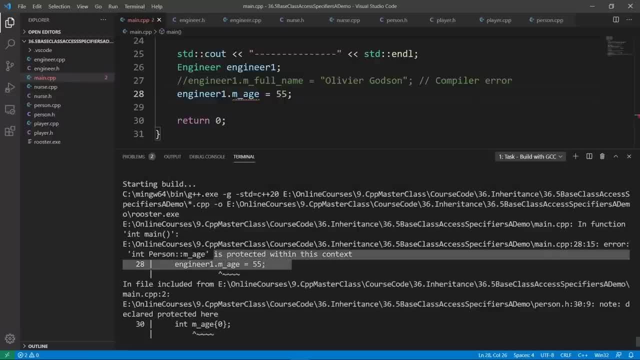 our error. we're going to see that m age is protected within this context, so we can't use it at line 28 of the main cpp file. this is going to give us a compiler error. let's do that. we're going to say that here, and if we try and access the m address member variable. 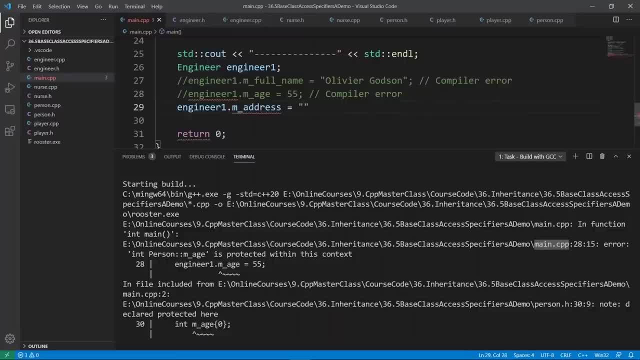 that's not also going to work because this is even more restricted for access. it is private to the base class, so we can't access it from a derived class directly. we can't even access that from the outside. so you should really know this. so if we put in some junk data here and try to 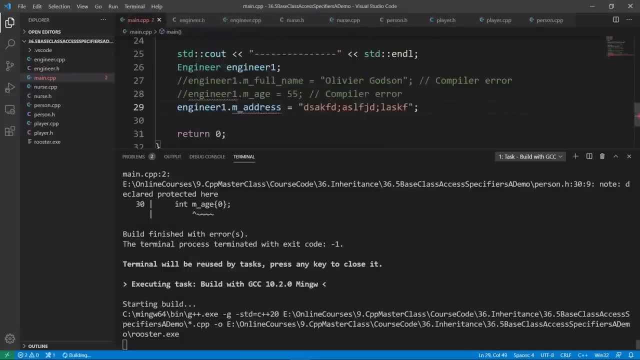 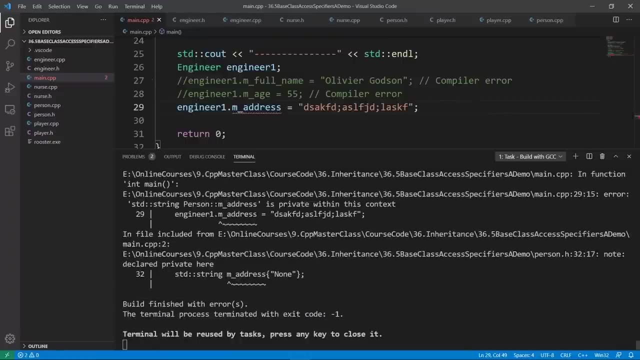 build. this is going to give us a compiler error that says that this is not accessible from the main cpp file, like we are trying to do on line 29 here. so we're going to get an error and the error is going to say: m address is private within this context and the offending line is at 29 of the main. 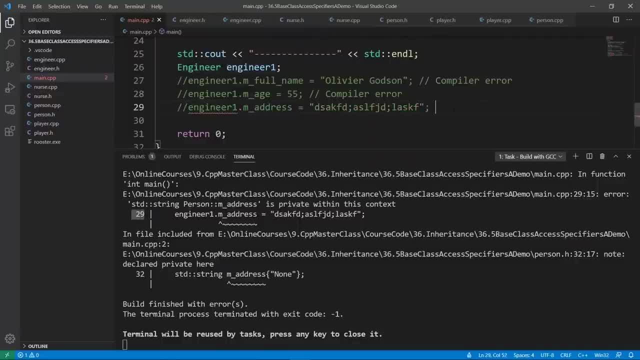 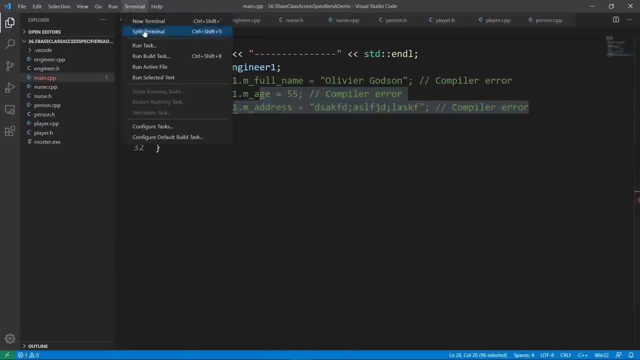 cpp file. we're going to take this out and we're going to say that this is going to give us a compiler error. this is really all i wanted you to see in this lecture, and before we wrap this up, let's try and build again and make the error go away, because i don't like to leave you with code. 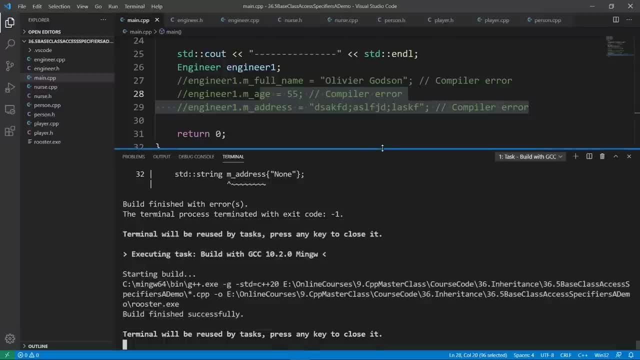 that has compiler errors and the build is good. and this is really all i wanted you to see in this: that you can do all kinds of inheritances in your c plus plus code. you can do public inheritance, you can do protected inheritance, you can do private inheritance and we had a chance to look at all. 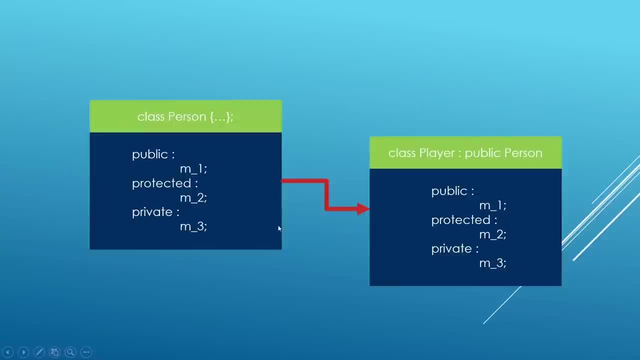 these scenarios in this lecture. here the message is the same as we saw in the last lecture: if you do public inheritance, anything that is public and the base class is going to stay public in the derived class. anything that is protected is going to stay protected. anything that is. 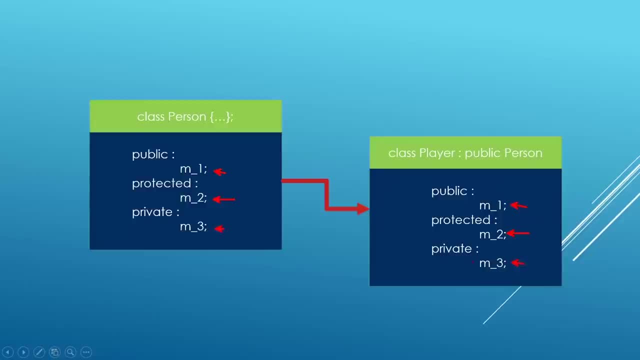 private is going to stay private, and this is really misleading in a way. the private data from the base class is not going to be private to the derived class. it's going to stay private to the base class. so if you try to use this in any way from the derived class, you're going to 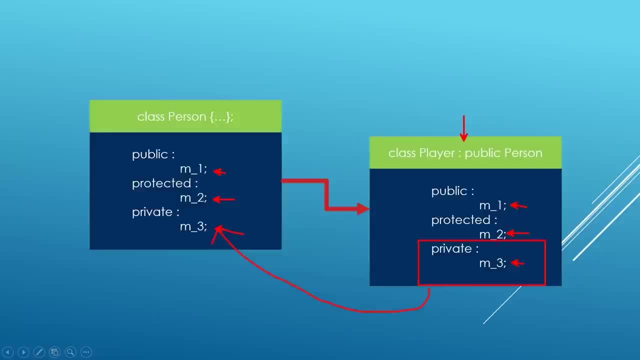 get compiler errors because you can't access that even if it is part of you. player has a person part of it, but it can't access private members from the base class. you should really know this. we have seen that we can also do protected inheritance and that's going. 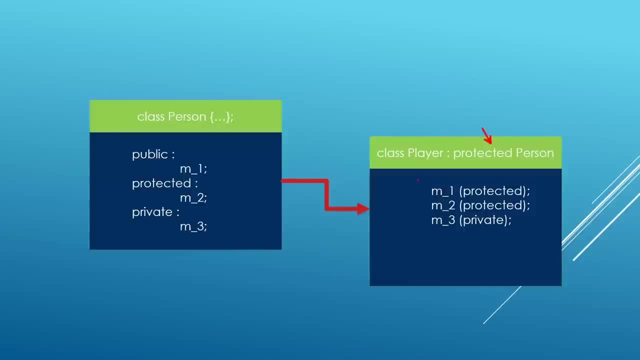 to constrain events to have the highest level of access to be protected. so anything that is public is going to be stripped down to protected access. anything that is protected is going to stay protected. anything that is private is going to be private to the base class. you should really. 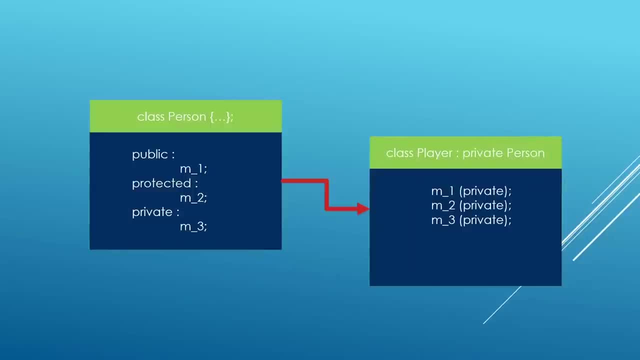 make this super clear. we can also do private inheritance, as we saw, and this is going to strip down the highest level access to be private. so anything that is public is going to be constrained to be private. anything that is protected is going to be inherited as protected. 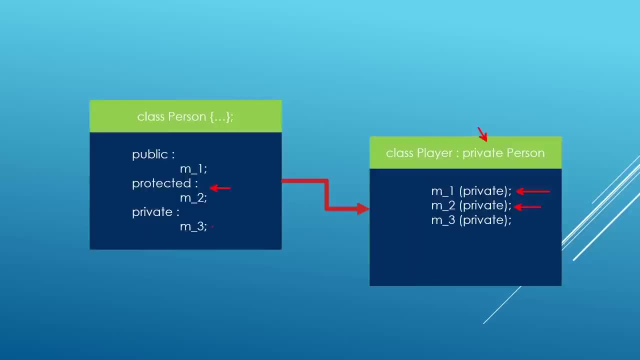 to the player class, but anything that was private in the base class is going to stay private to the base class. even the player class won't have access to this member directly. if we really need access to private data from the base class, we might go through public getters or 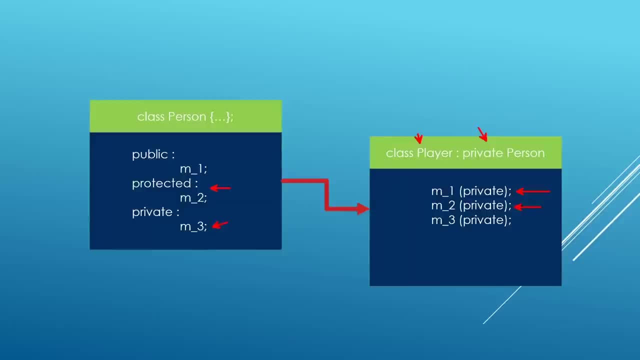 get access to private data from the base class, but we can't access m3 directly and use it from the derived class. that's going to give us a compiler error. this is really all i wanted you to see in this lecture and i hope you find this interesting. we are going to stop here in this. 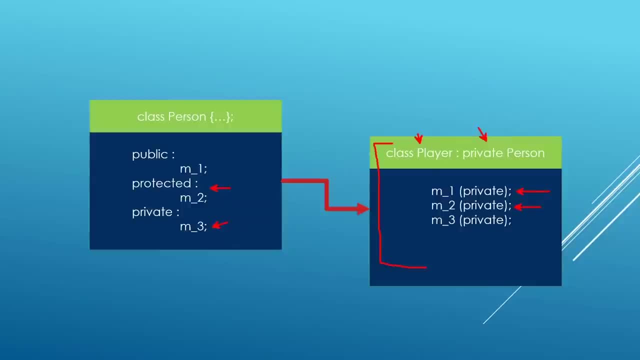 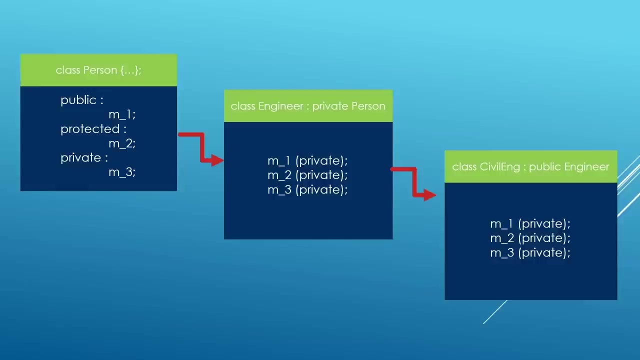 lecture. in the next one we're going to try and zoom in on private inheritance and show you some things you really need to be careful about. so go ahead and finish up here and meet me there. in this lecture we're going to zoom in on private inheritance and we're going to see that the class that does private inheritance is really selfish. 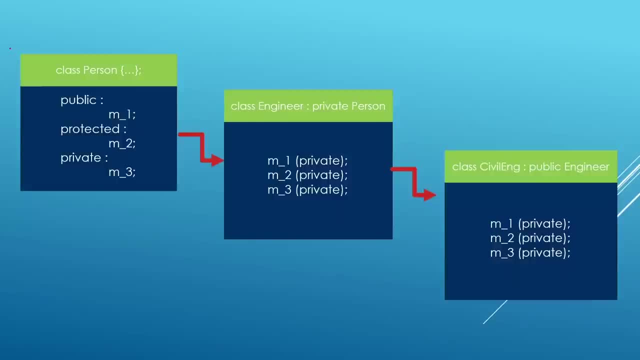 here is a simple structure we will be using in this lecture. here we will set up a person class which is going to act as our base class. we are going to inherit from this class privately and create an engineer class, and what this is going to do? it's going to take everything from the class. 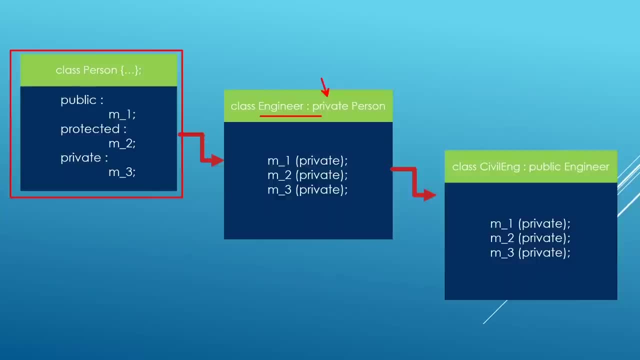 person and make it private to the engineer class. so the m1 member variable, which was public in the base class, is going to be private to the engineer class. this is what we have here. the m2 member variable, which was protected, is going to become a private in engineer. that's what we have here. and the m3 member variable, which was private to person. 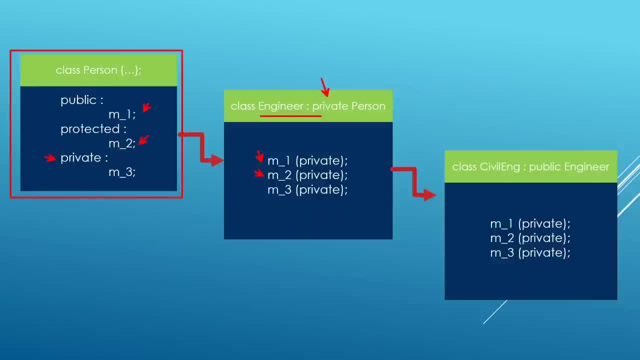 class is going to stay private to person in the eyes of engineer. this is the situation we have here. so the problem is going to really show up here when somebody else tries to inherit from engineer. because m1 and m2 are now private to engineer, they will be inherited but still inaccessible to the civil engineer class. here m1 and m2 will be. 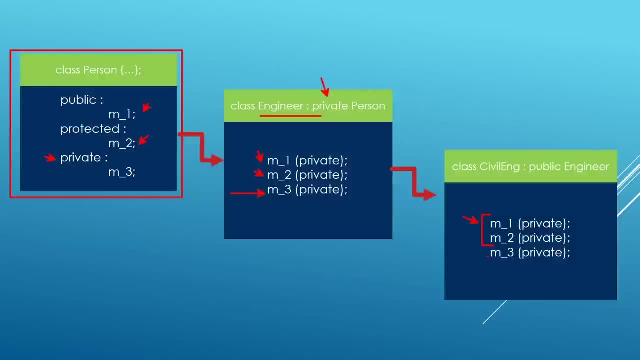 private to the engineer class, but m3 will be private to the base class, which is person. so hopefully you can see the message that if a member variable is private, it can't be inherited in any way, it doesn't matter which kind of inheritance you do. so, starting from engineer, which has made m1 and m2 private to itself, it's no longer possible to 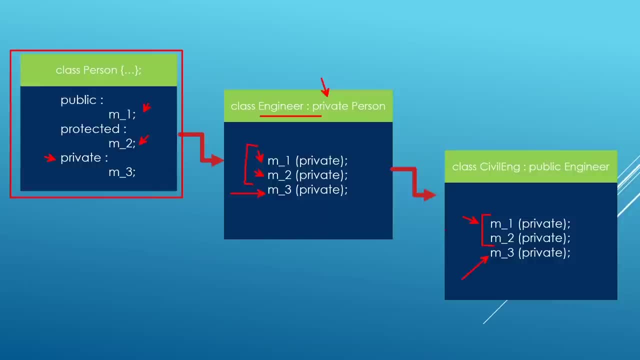 forward these guys down in the inheritance hierarchy. another way to look at this is to see that the engineer class is really selfish. it is saying: i am going to take everything i can get from my parent classes because i am the engineer class and i am going to take everything i can get. 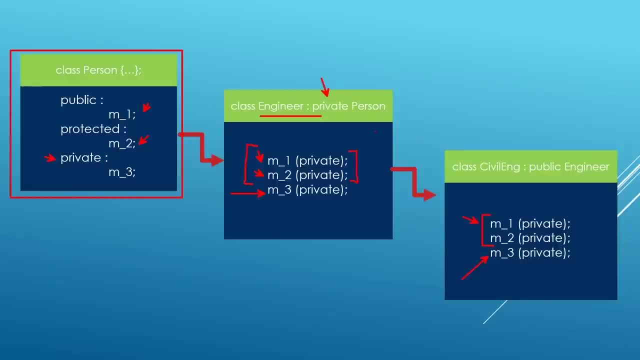 from my parent classes because i am the engineer class and i am going to take everything i can get from my parent classes. because i am the engineer class and i am going to take everything i can get inheriting privately. but nobody else will be able to take things from me because i'm going to make 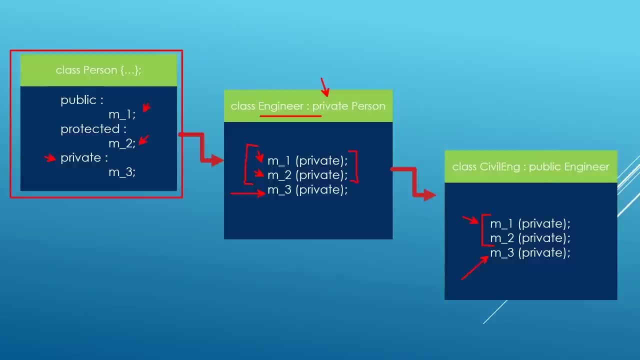 them private to myself. so even if civil engineer is doing public inheritance, that's not going to give him any access to these member variables which are now private to the engineer class. hopefully you can really see this and private inheritance is going to really constrain what you can forward it down to other classes. 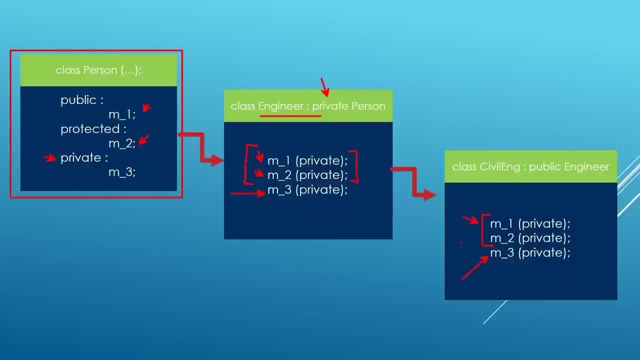 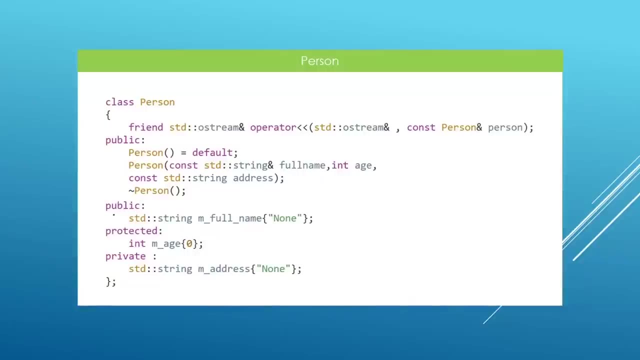 hopefully you can really see this, and private inheritance is going to really constrain what you can forward it down to other classes that are going to be inheriting from you. this is the message i am trying to convey here. okay, so here is the same example in code: we have our person class. it's going to have our. 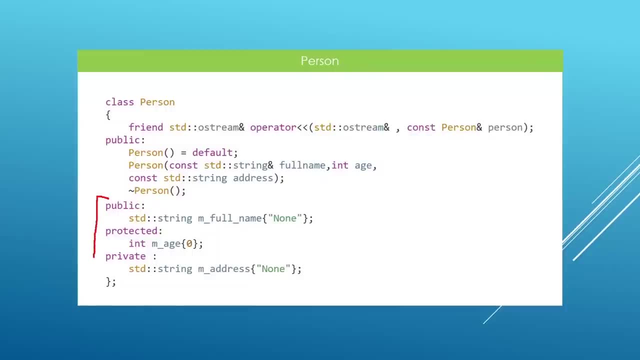 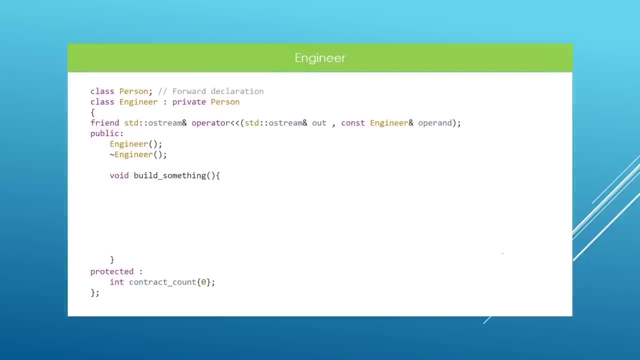 member variables. we're going to have the full name, the age and the address. they are going to have public, protected and private access. we are going to inherit from person and create our engineer class. we are going to privately inherit from person and this is going to take. 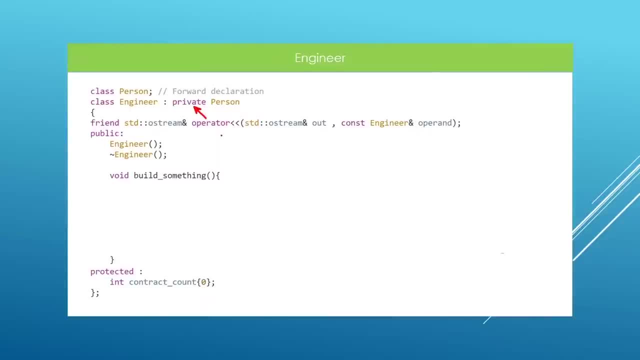 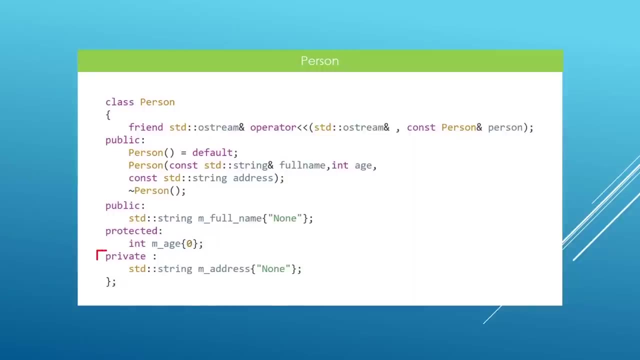 everything we got from our engineer class and we are going to take everything we got from our person from person and make it private to the engineer class, and one exception is going to be what was already private to the base class, which is our person class. here this is going to still 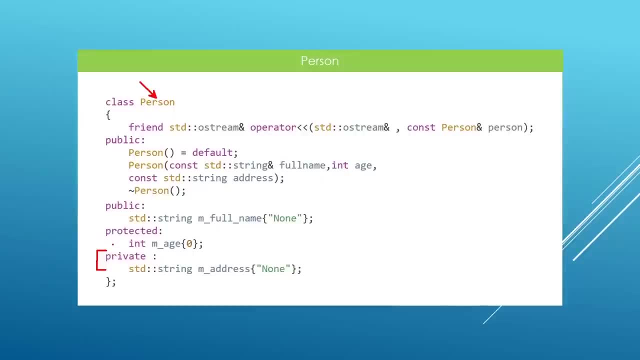 stay private to the person class, regardless of what kind of inheritance you do from person. but any other thing, if we have any member variable which are public or protected, or even if we have some member functions which are public or protected, anything right. so for instance in theLawn class, right, this is going to stay private to the 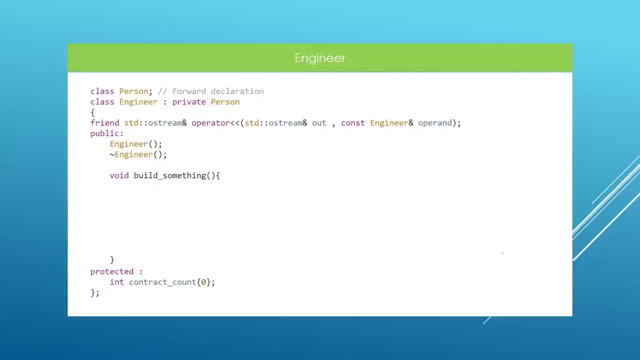 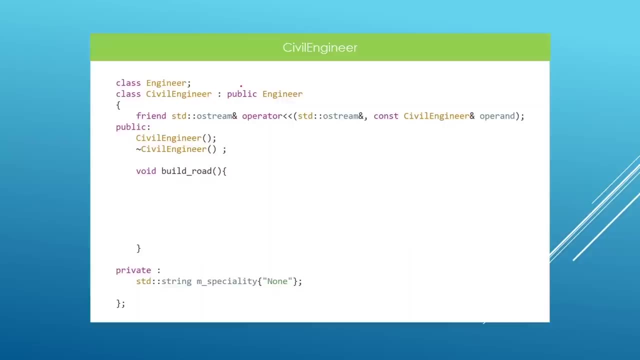 engineer class because we do not have a plus advantage here today. everything here is going to be private to the engineer class because we have done private inheritance here. so if we inherit from engineer and do any kind of inheritance we are going to do the most relaxed kind of inheritance which is going to keep the kind of access we had in the base class. but 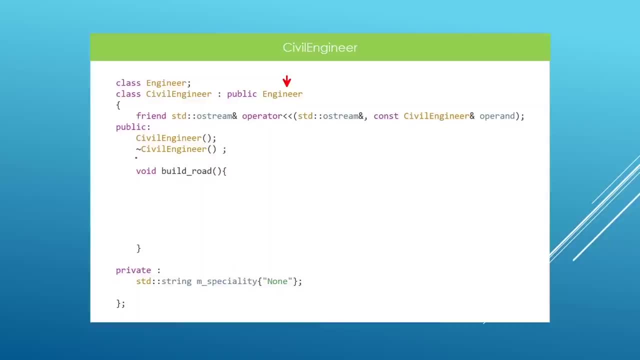 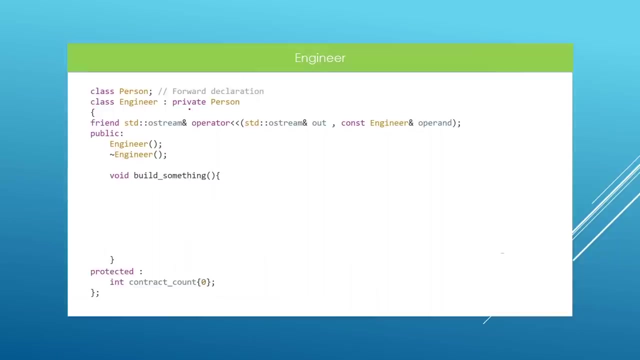 really not going to have any access to any member variable or member function that is inherited from the engineer class, and we are going to see this in a minute when we hit visual studio code. so, again, if a class is doing private inheritance, it's really another way to say this class is selfish. 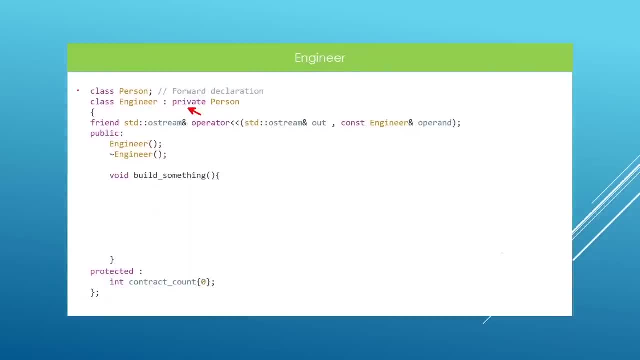 it's going to take everything it can from the parent class, but it's not going to forward nothing to downstream inheriting classes, and this is the setup i really want you to understand here and only do private inheritance when you want this kind of behavior. now that you know this, 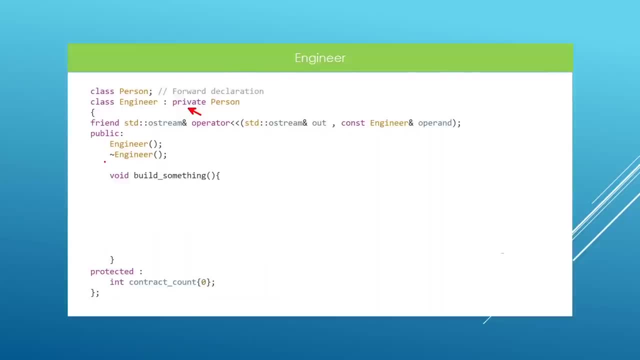 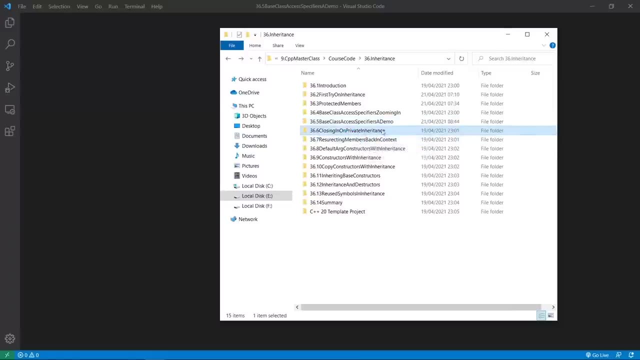 we're going to head over to visual studio code and play with this a little more. here we are in our working folder. the current project is closing in on private inheritance. we're going to zoom in on this and really understand the effects of doing private inheritance. we're going to grab the code from the previous lecture and we're going to grab the engineer. 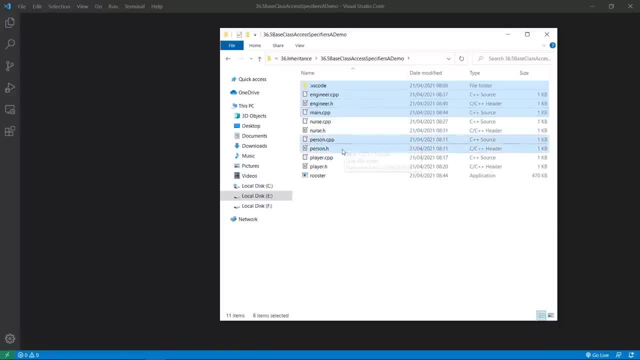 and the personal class. these are going to be our starting point here. make sure you grab the vs code folder if you are using vs code with this course. that's going to give you the basic settings we need to do our c++ program. i am going to copy these guys down and put these in our 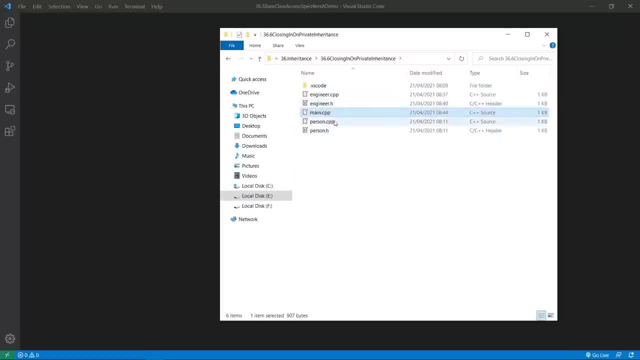 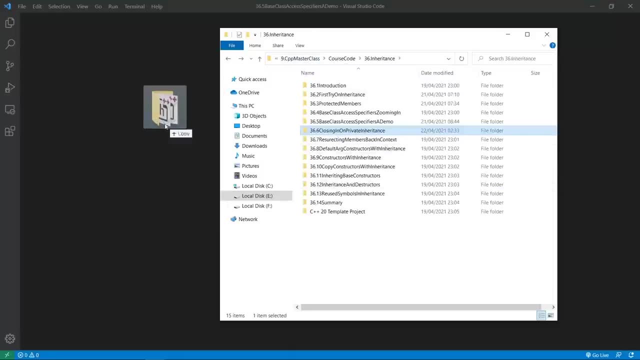 current project and again, make sure you have the main Cpp file file, the person class and the engineer class, and these are going to be our starting point. so we're going to open this little guy in visual studio code by dragging and dropping. here we're going. 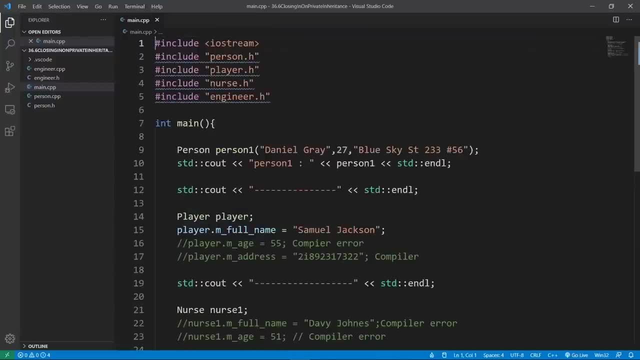 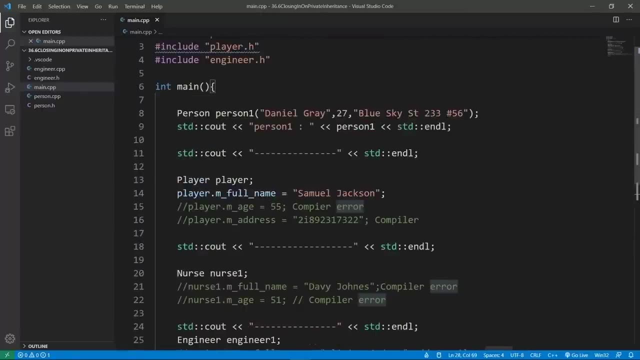 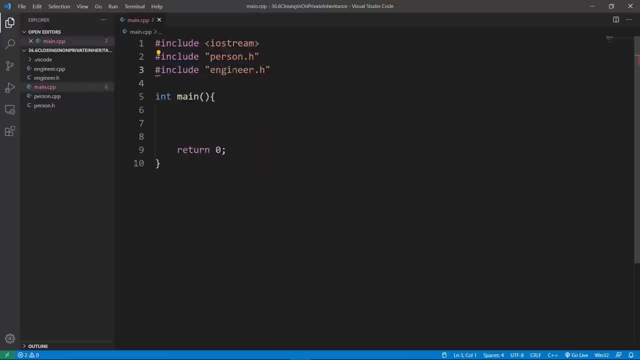 to look at our main cpp program. we are not going to include the nurse because we don't have this included here and we can really take out everything we have in the main function. we're going to be adding our own thing here. we also don't need the player class here. 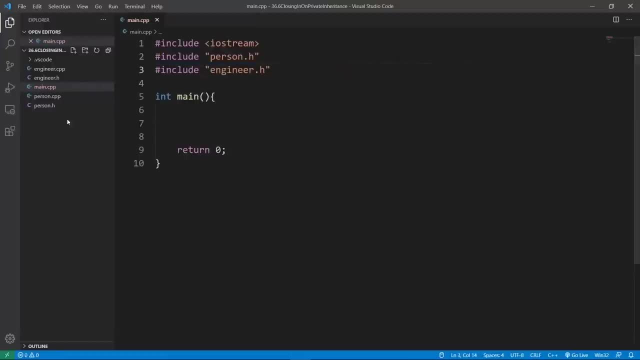 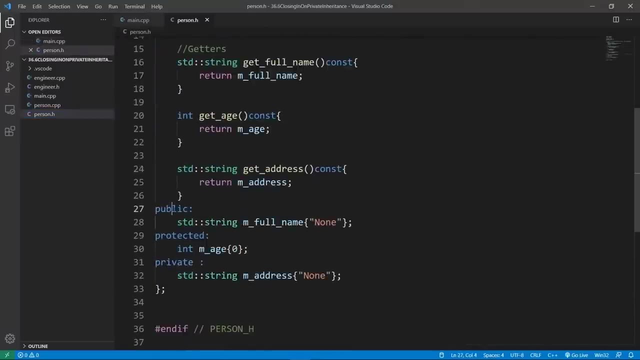 we're just going to be using person and engineer. let's look at the person class. it is going to have the member variables that we expect. we are going to have a public member variable- the full name- a protected member variable- m- age- and a private member variable- m- address. here, 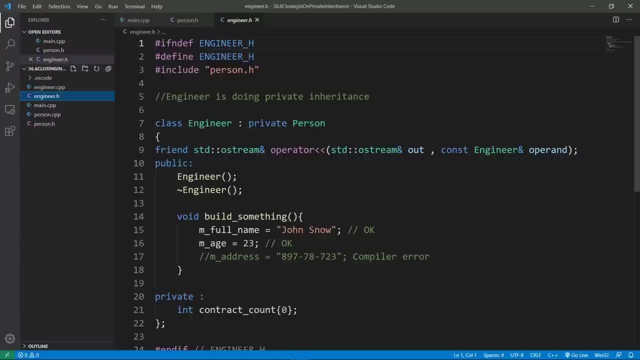 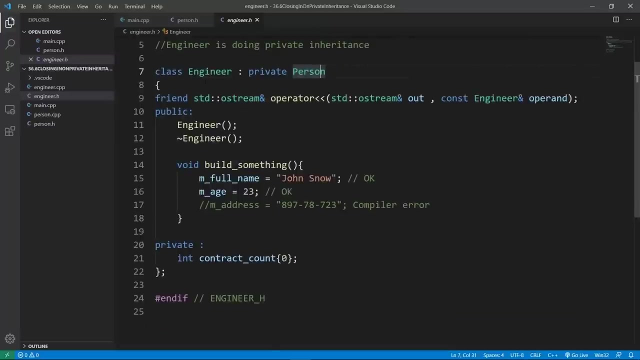 we are going to create an engineer class which is going to privately inherit from person, so it is going to make everything private to itself. the engineer class is going to have a person part in it, but the member variables we get from the person class are going to be stripped. 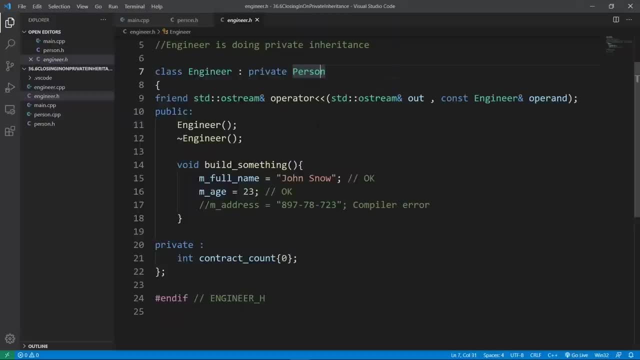 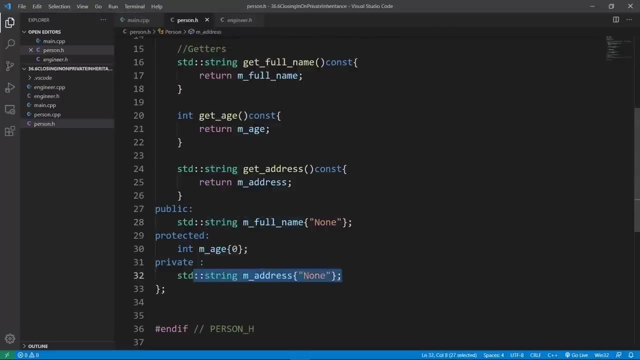 down to private access level, except for the member variables which are already private in the base class and that happens to be the address. so it doesn't matter which kind of inheritance you do, the m address member variable is going to still be not accessible to inheriting classes. this is going to still be private to the base class. 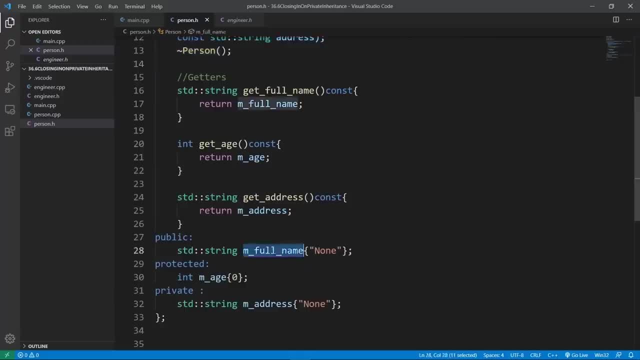 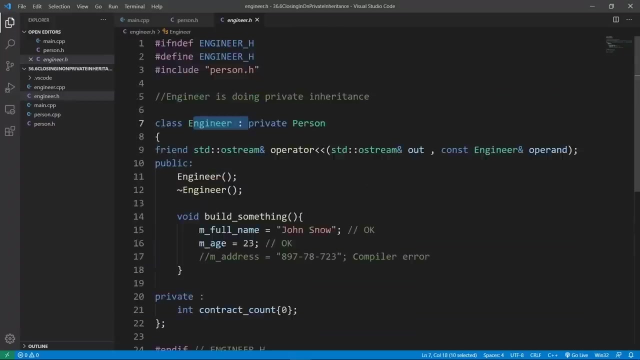 which is the person class here. so the full name is going to be stripped down to private access level. in engineer, the edge is also going to be stripped down to private access and these are going to be private. now to the engineer class, and any class that tries to inherit from engineer is not going. 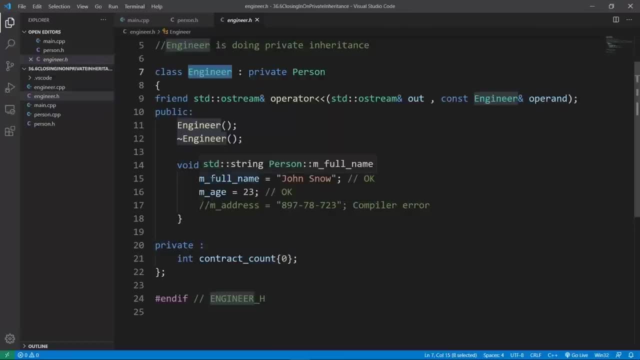 so if we do any kind of inheritance from engineer, we want to have access to full name. we want to have access to m age, because these are going to be private to this class here. this is the setup we want to understand in this lecture. so what we're going to do, we're going to set up a new class. 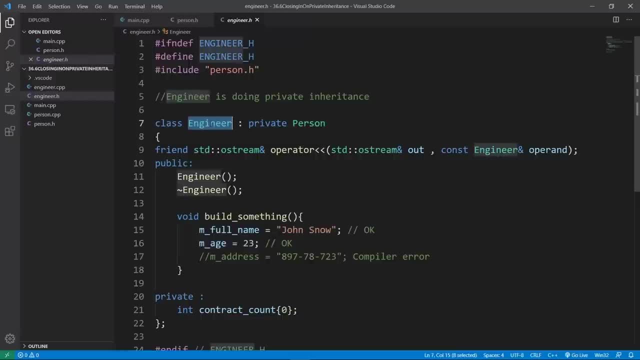 which is going to inherit from our engineer class and it is going to do public inheritance and we're going to see how this works. we're going to create a civil engineer class which is going to inherit from engineer. so we're going to create a civil engineer class which is going to inherit from. 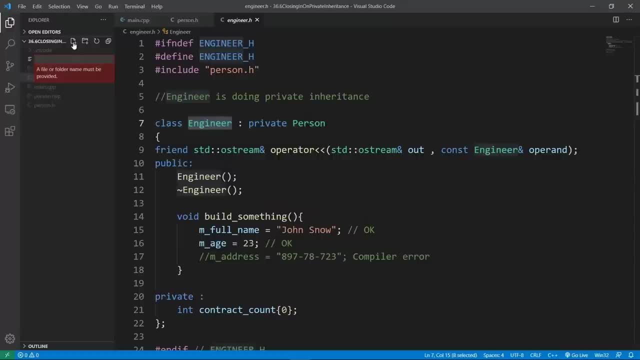 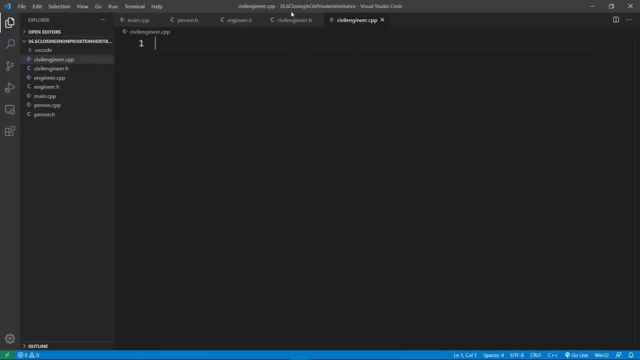 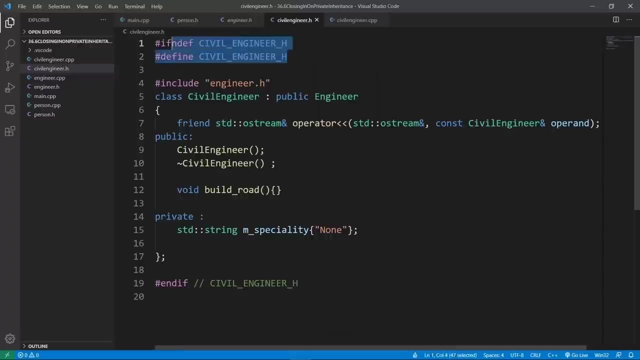 engineer. so let's do this. we're going to create a header file for our civil engineer class and we're going to create a cpp file. we are going to head over in our header file and put in the class. it's not going to be anything sophisticated, we're just going to have in our include guard. we're. 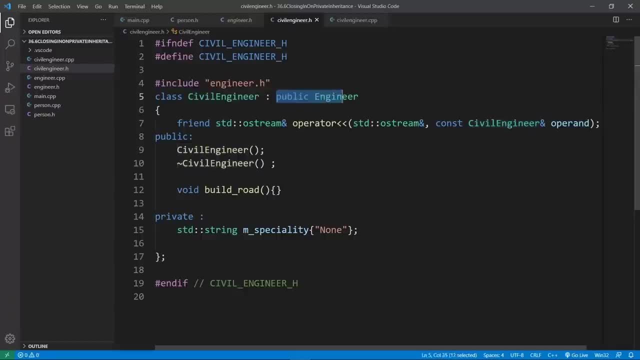 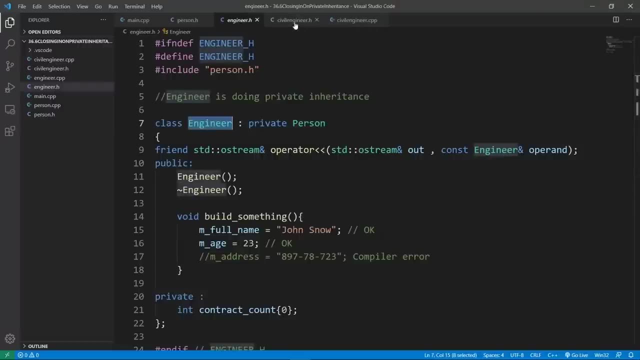 going to create a civil engineer class which is going to publicly inherit from engineer. but remember, everything was made private to the engineer class. so, even if we're doing public, in this case, we're going to have a civil engineer class which is going to be private to engineer. 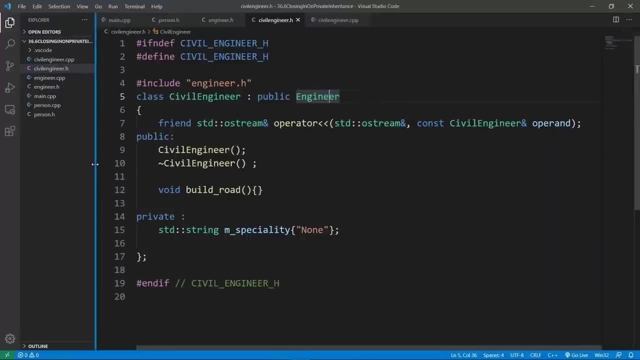 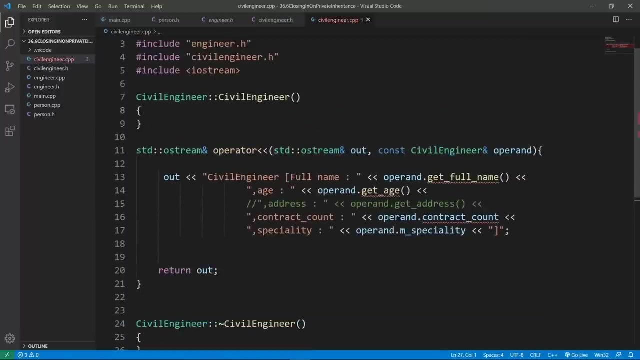 the h is going to be private to engineer and engineer won't have any access to these guys. but before we really play with that, we're going to put in our implementation in the cpp file. so let's put in the code here. we're going to put in the implementation and we're going to have our 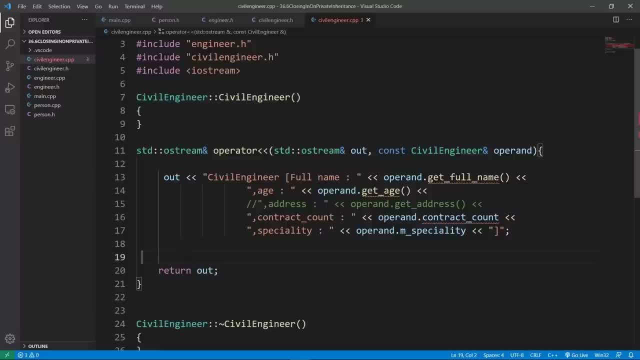 constructor in place. but notice what happens on our output stream operator. the output stream operator front of the civil engineer class, so it should have access to anything we have in our civil engineer class. but notice what is happening here. the get full name method is not working because 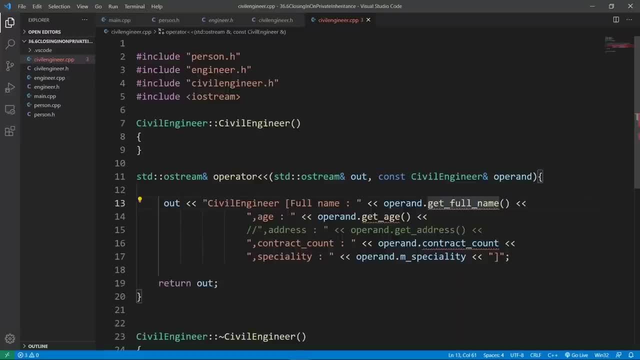 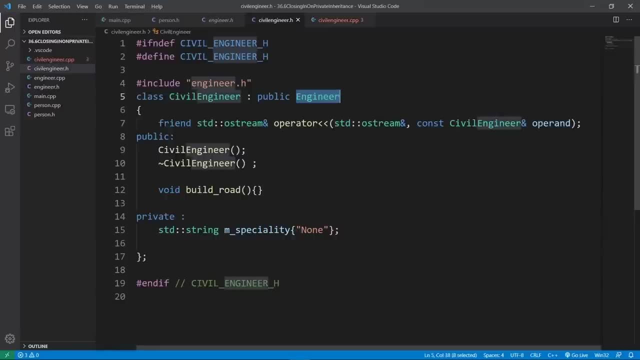 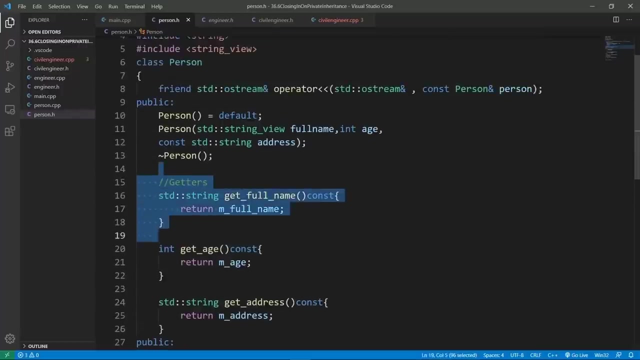 it has been made private to the upstream class, which happens to be our engineer class, and we can't really access them, even if we know that they are really part of the interface of the person. we have them as public members of the person class, but when the engineer class did private. 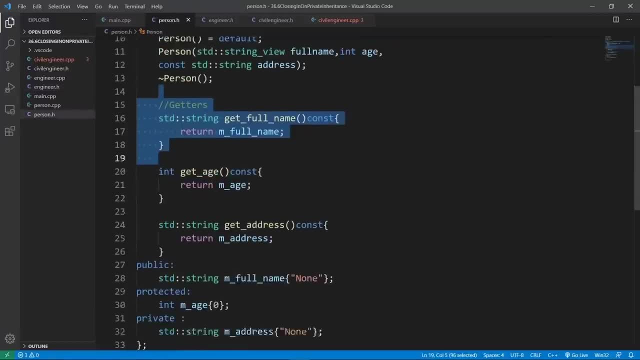 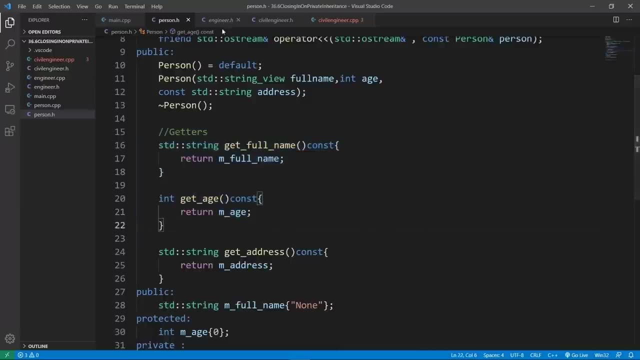 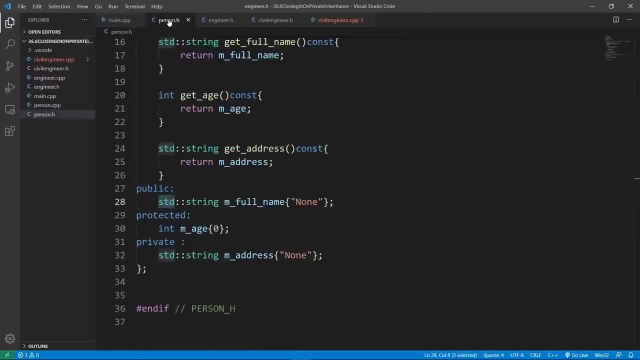 inheritance, it made everything that is not private to person private to itself. so these gators are going to be private to engineer. when the engineer does private inheritance, the member variables, which are public and protected, all these things are going to be stripped down to private access level. so they are going to be 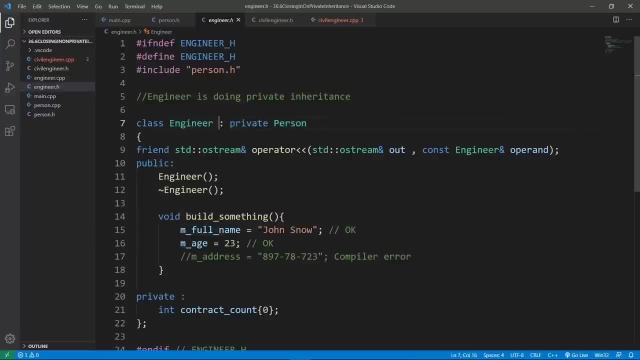 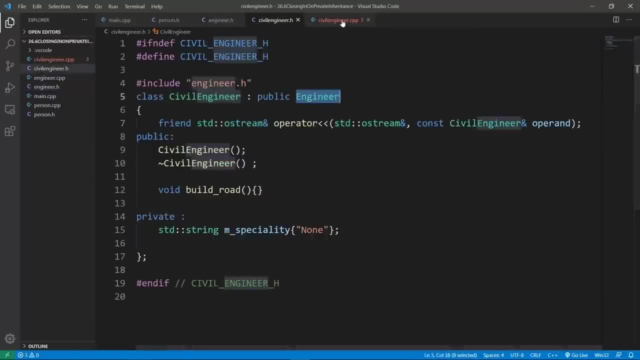 private to engineer and any kind of inheritance you're going to do is not going to change that. they are going to be inherited as private to the engineer class. that's why we can't even call them from a function which is a friend of our civil engineer class and we know that. if you mark 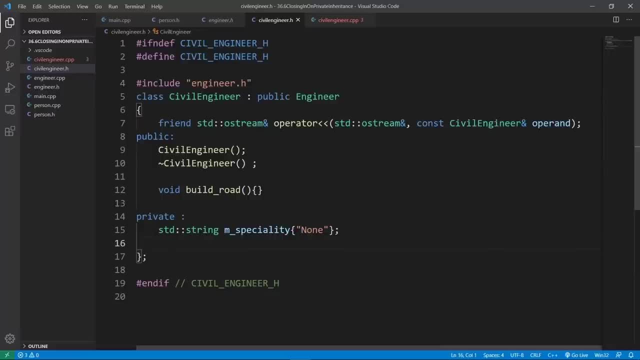 something as a friend. it's really going to have access to anything you have, including private members, but we can't call any of the members from the engineer class because it's not private to the engineer class. this is what i want you to see if you do private inheritance. 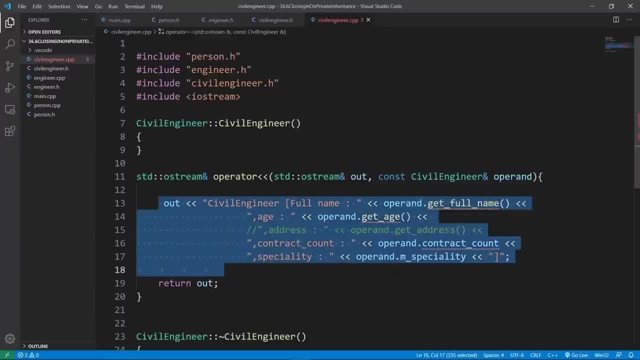 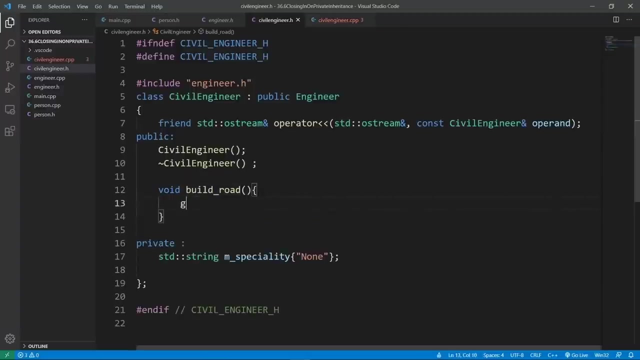 this is going to really strip down anything from the upstream class and make that private to the class that is doing private inheritance. this is the message here and again. if you go in any method of the civil engineer class and try to do any kind of access, for example calling the gate full name- 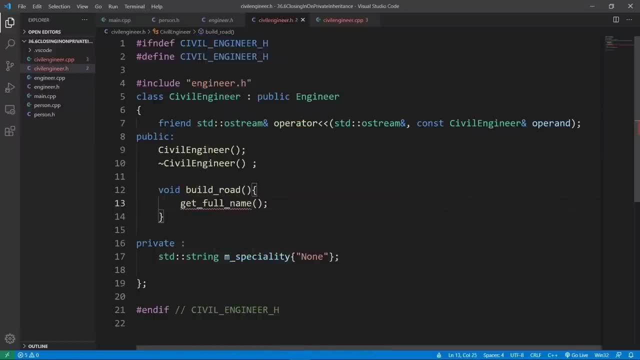 method is not going to bode well. we're going to see that this is not accessible here. if we try to access m full name, for example, change this to be something else, let's say daniel gray, this is not going to work. if you try to access mh and change it to 45, for example, 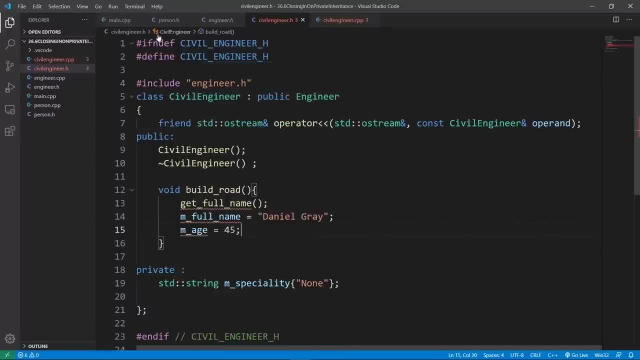 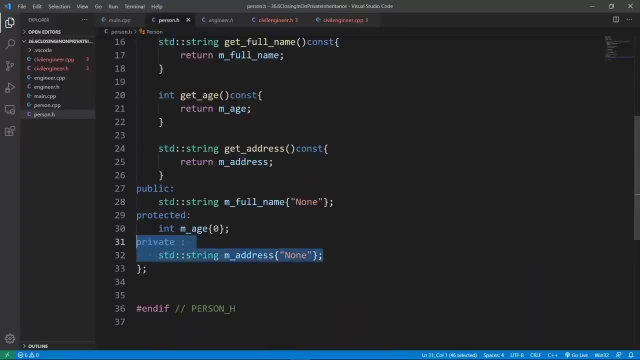 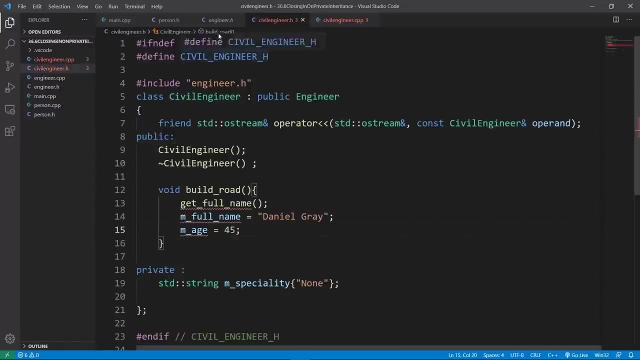 this is not going to work. we already know that the address is private to person, so we shouldn't really try to access it because it is inaccessible, regardless of any kind of inheritance you do. but the members that were public from person be accessed from any class that is inheriting from person, even if we know that these things 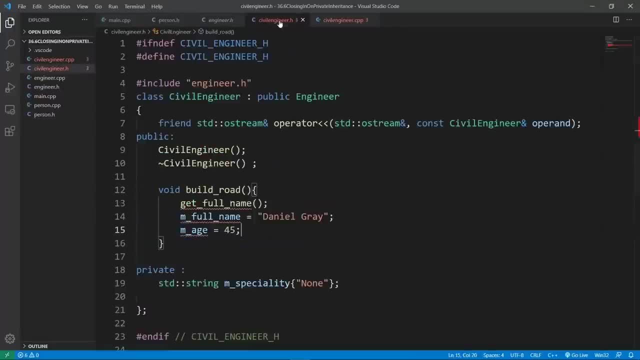 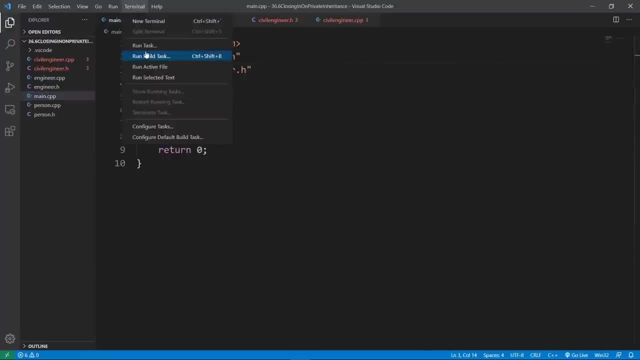 are public or protected in the person class, and this is really what i want you to see. if we try and build our program, we're going to get a bunch of compiler errors saying that we can't access these guys from our civil engineer class. we are going to use the 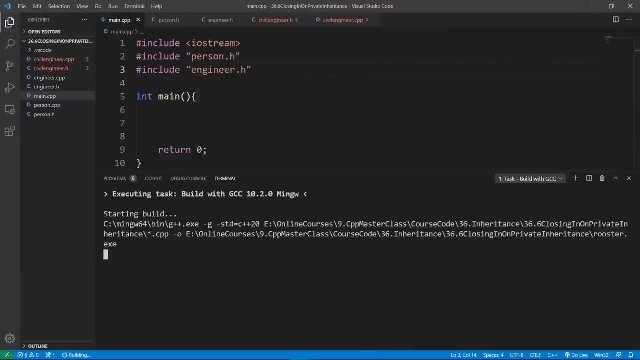 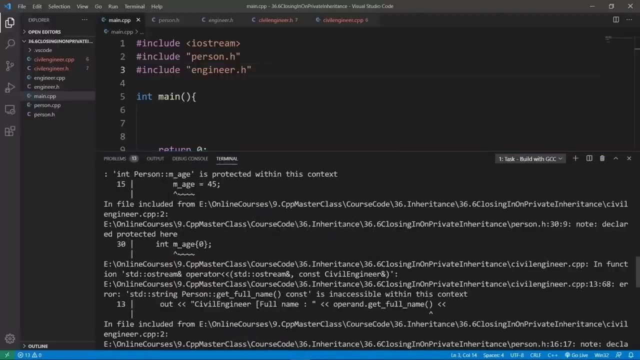 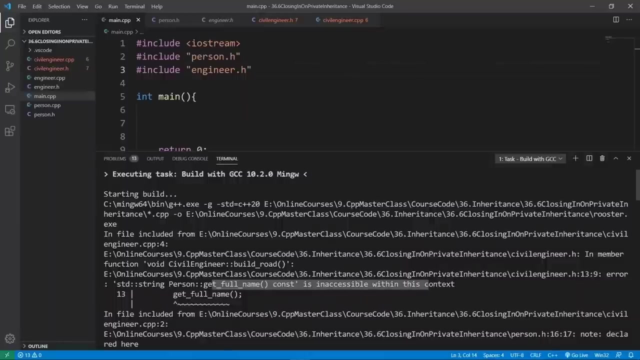 gcc compiler here because it is our favorite and we're going to see our compiler errors here. okay, so we're going to get a bunch of errors. let's go up and see all of them. we're going to get an error saying that get full name is inaccessible within the context of the c4. 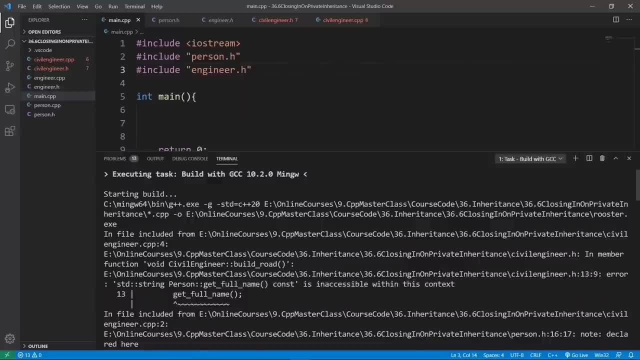 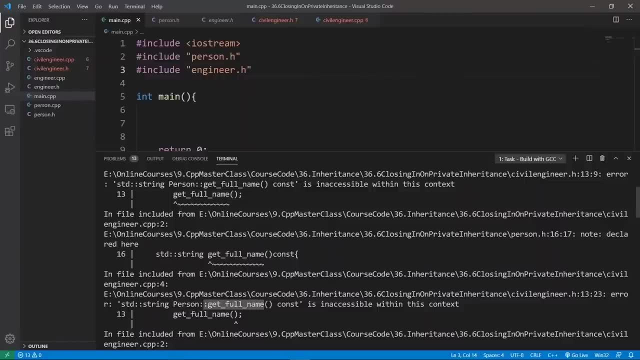 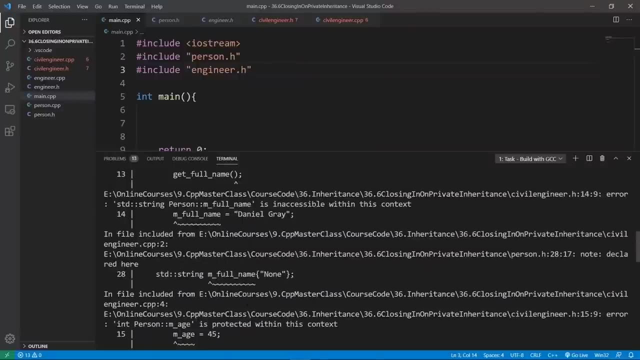 engineer header class at line 13. we are calling this method. that's not going to work. we have another error here, saying that the get full name method is not accessible from line 13 of the civil engineer header. it is really the same error but if we go down we see that we get a bunch of other errors we have 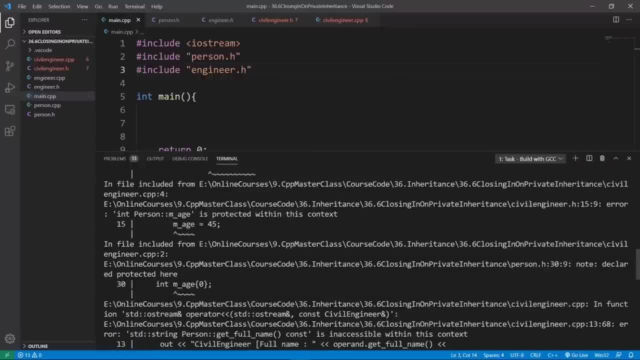 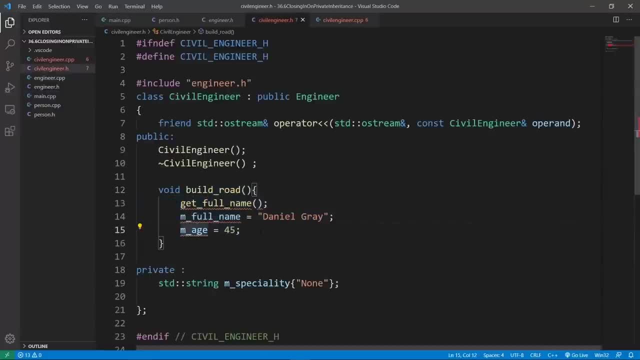 m full name, which is not accessible. we have m age, which is not accessible. we can't really do these kinds of fans from the civil engineer class because all these are going to become private to the upstream class that did private inheritance. so let's take these out and show you that, even if 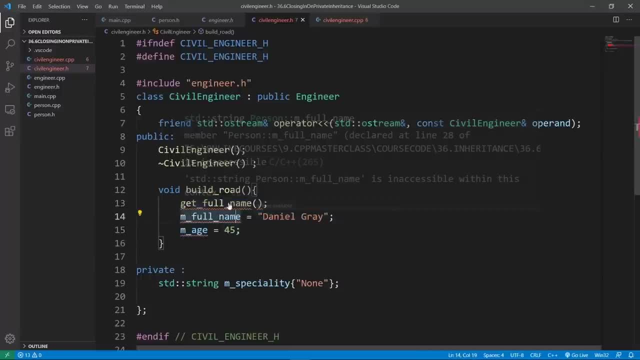 we can't access these guys. they are still part of our civil engineer class and we're going to use a debugger to do that. i am going to take out these things, or i can comment them out and say that they are going to give you compiler errors. i think this is going to be more descriptive, so 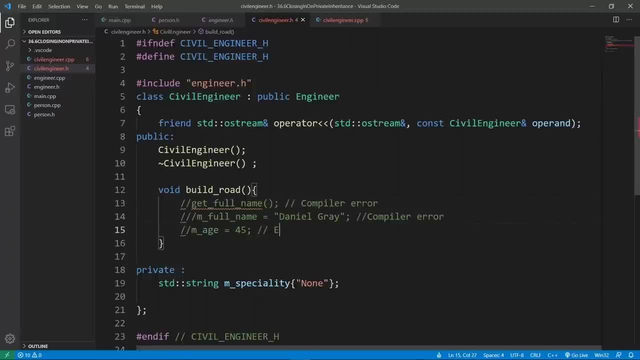 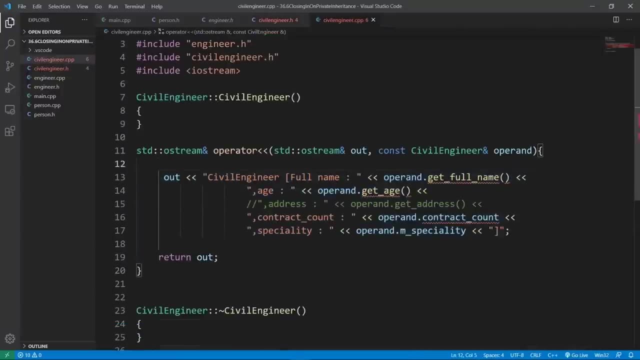 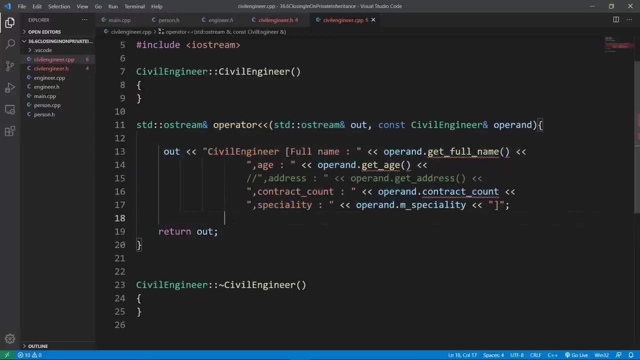 let's say compiler error, and access to the edge is also going to give you a compiler error and we're going to go down and show you that we're also going to have the same problem in our output streamer operator. so if you really want your output stream operator to work here, 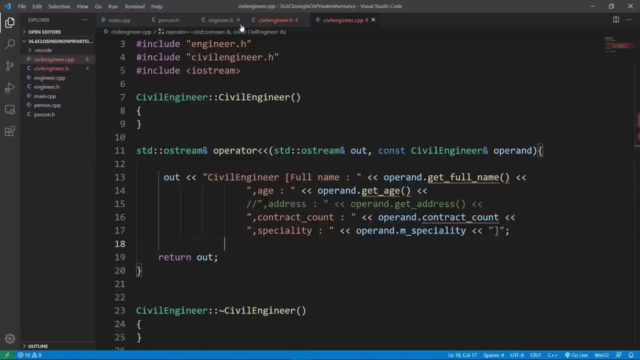 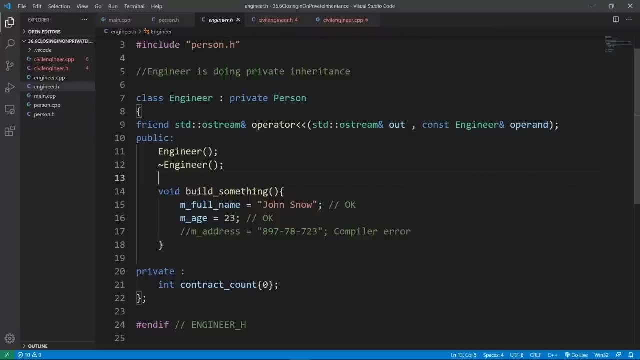 what you can do is put some public members in the engineer class and make it give you access to the members that were eclipsed to private access in this class. here, for example, you can return the full name. you see that we can access that. here you can return the age, but 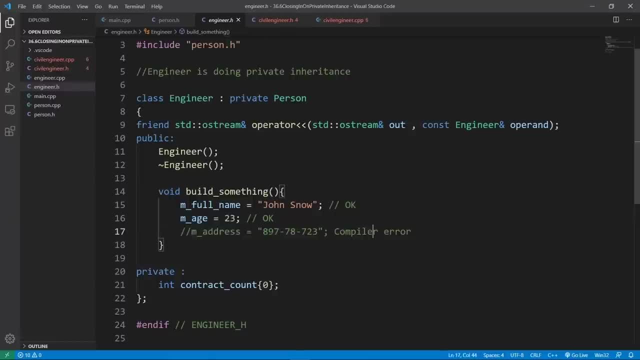 you still don't have access to the m address member variable because this is private to the person class. but i really don't even want to do this because doing this kind of design is sign of bad design in the first place. so if you need to do those kinds of gators and forward them down to 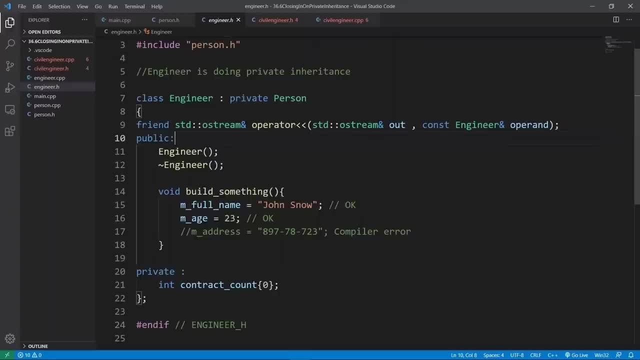 inheriting classes. why not change the design in the first place and not do private inheritance here? for example, if you change this inheritance to protected or public, these members are going to be directly automatically forwarded the inheritance to the public. so if you change this inheritance to private, you can put in public gators that are going to be forwarded down to any inheritance class. 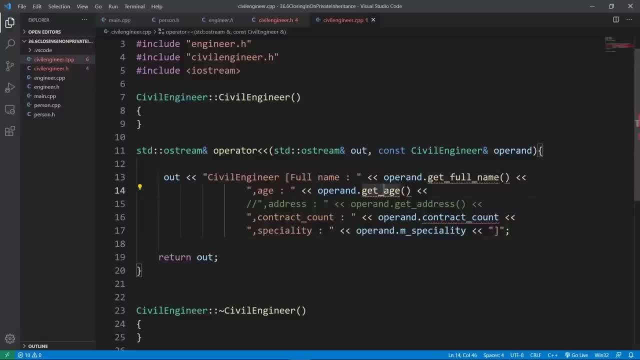 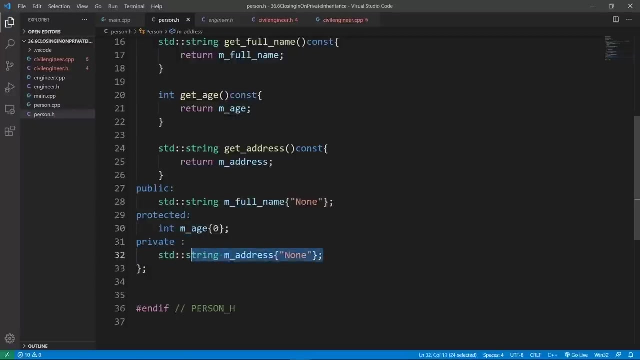 so just note that you can put in public getters that are going to give access to the full name and age, but you still won't be able to access the address member from the inheriting class, because this is the design you achieve by marking something as private in the base class. if you want the 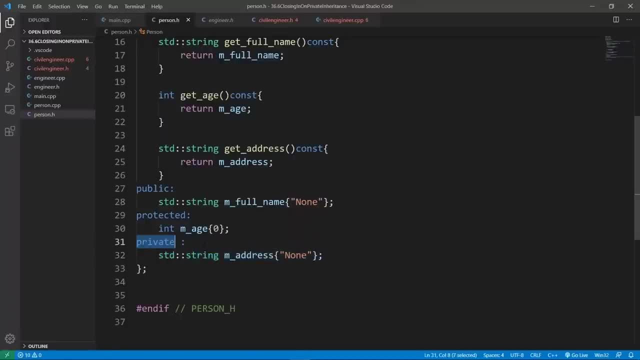 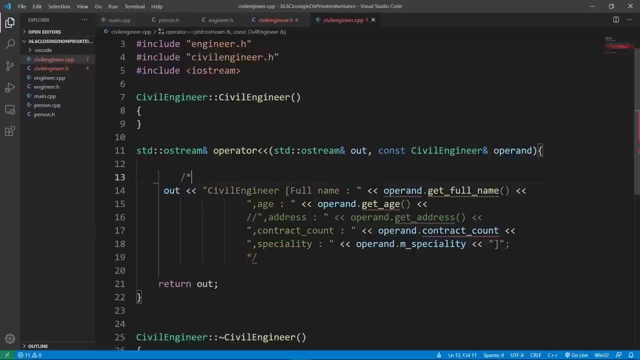 address to be forwarded down. you might change the access level we have here and maybe make it so. this is the ideas i really want you to grasp. i am going to comment out the offended code here because i want you to be able to build this program and see that, even if we can't access 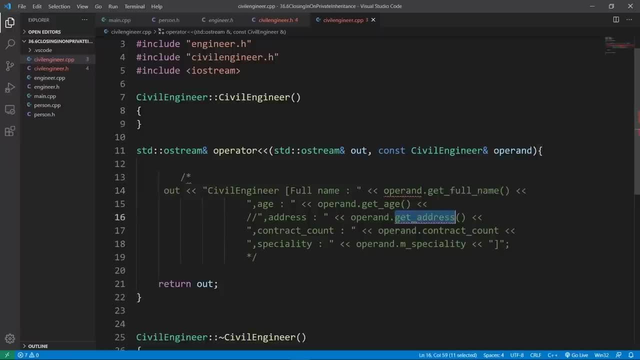 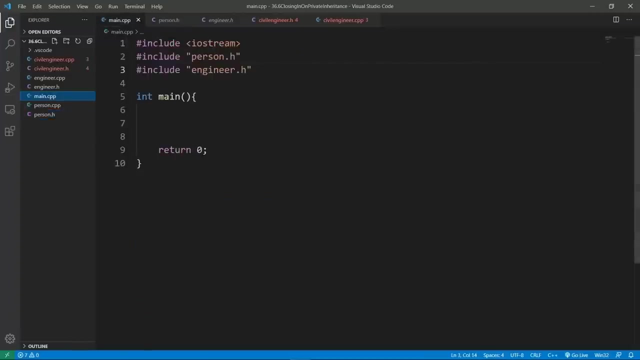 this: get full name and get address members from inheriting classes. they are still part of our interface. we just can't have access to them because of the choices we have made in upstream classes. so what i am going to do? i am going to go in my main cpp file and i am going to create: 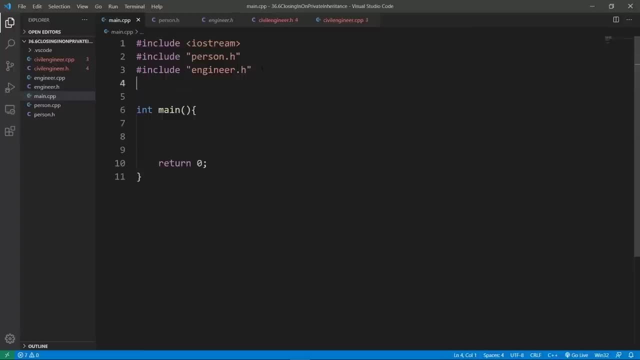 an engineer object. i will also include civil engineer here. let's do that, and i am going to create an engineer object and i am going to create a civil engineer object and i am going to just say: done here. and i am going to put a break point on 9, 12. we are going to use a debugger to really see. 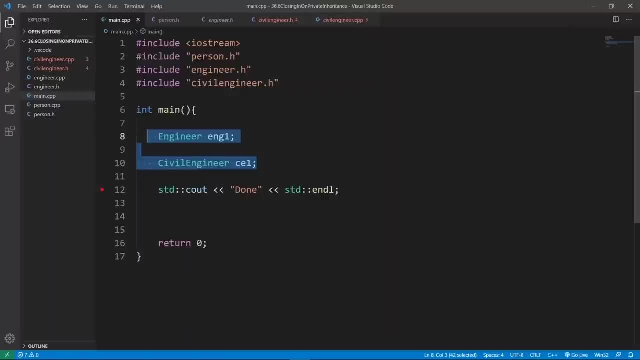 that engineer objects and civil engineer objects still have a person part of them. we just can't access the interface that was eclipsed by the engineer class. so we are going to hit the run tab here and we are going to start our debugging session by clicking on the green button here. 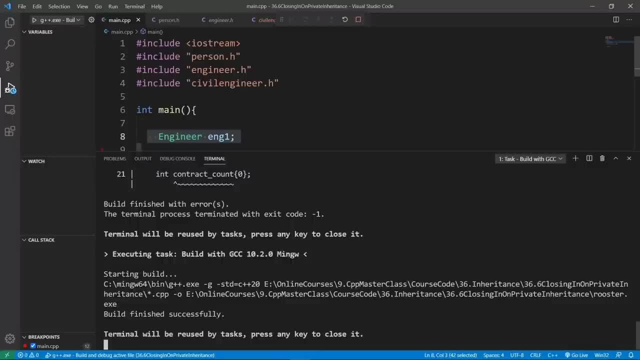 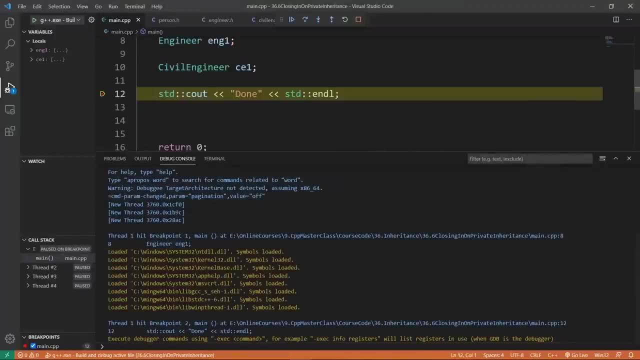 we are going to build our program and if the build is good, we're going to plug the binary that was generated into our program and we are going to start our debugging session by clicking on the debugger and we are going to hit our break point in a minute. once we hit our break point, we are 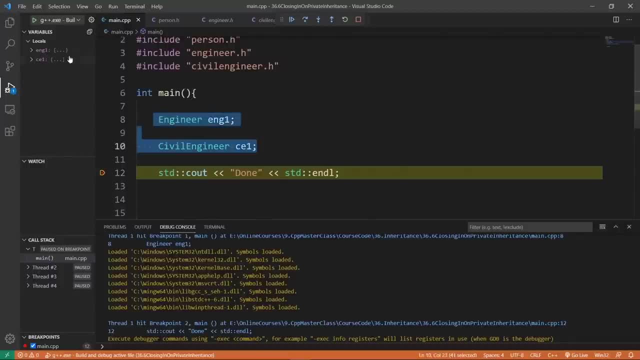 going to look at the local variables we have in the main function. we're going to see them on the left here. if we expand, we're going to see that we have an engineer- one object and we have a civil engineer- one object. if we look at our engineer, we're going to see that we have a 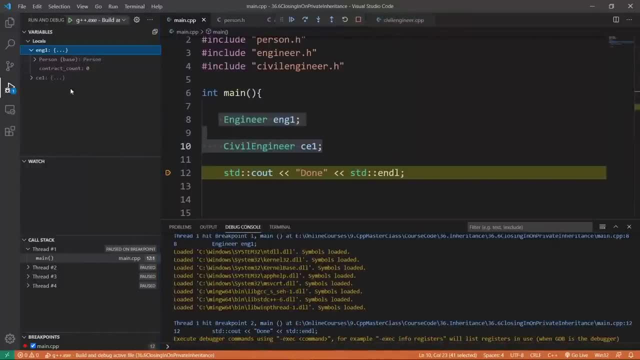 person part of this, which is our base class, and if we look at civil engineer, it's also to have a base of engineer. so any civil engineer is also going to be an engineer, but the engineer part of civil engineer also has a person part of that. you should really see this information. 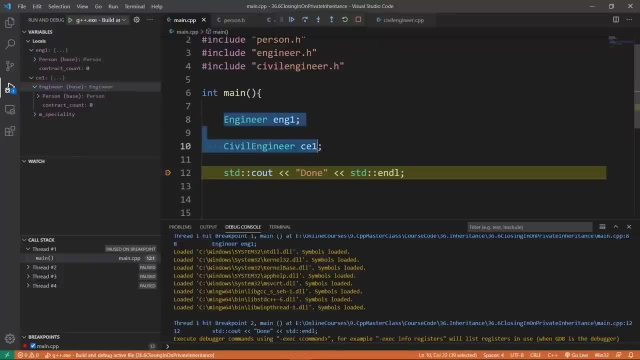 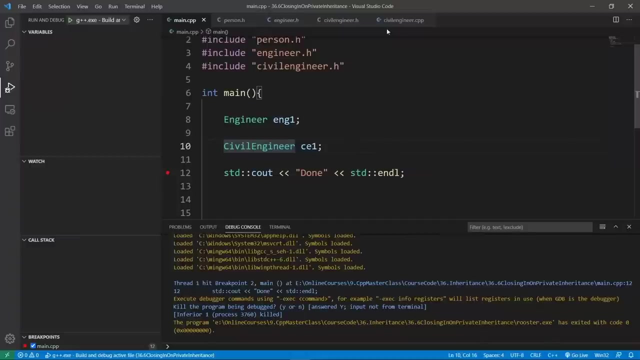 and the main message i want to convey here is that all these objects have a person part of them. we just can't access that part in objects of our inheritance classes because of the design decisions we have made. let's close this off now that you have seen this, and again, 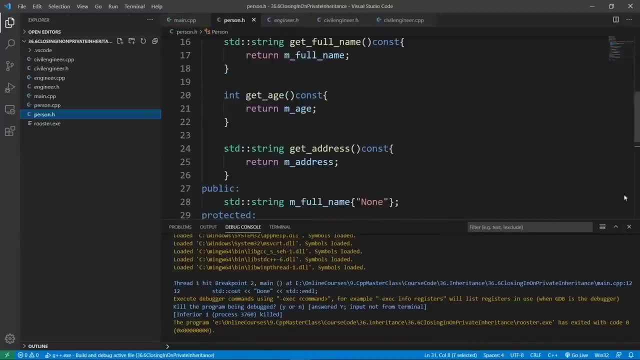 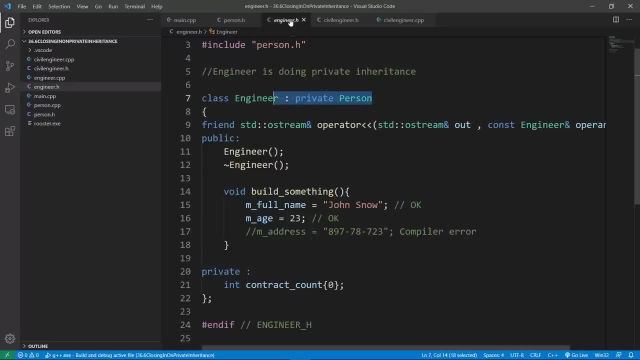 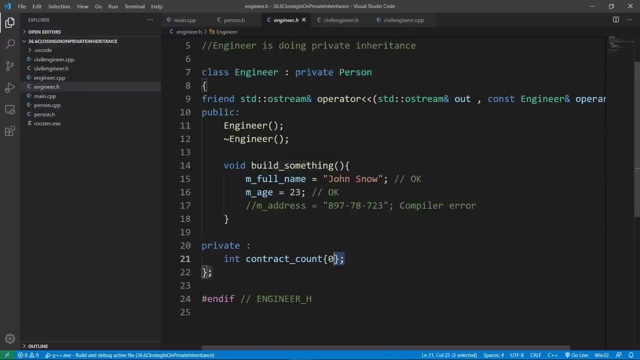 we are really working on this inheritance hierarchy. the base class is person and it's going to have these member variables. but if we do private inheritance from the person class, anything that is not public is going to be eclipsed down to private level access. so any other class that is going to inherit from our engineer class now 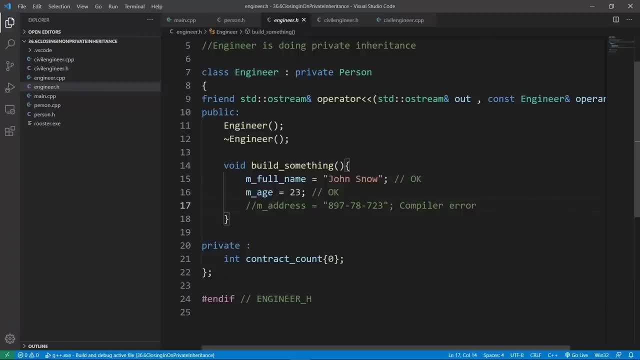 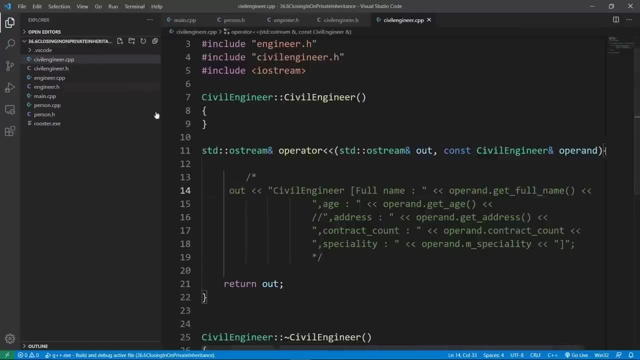 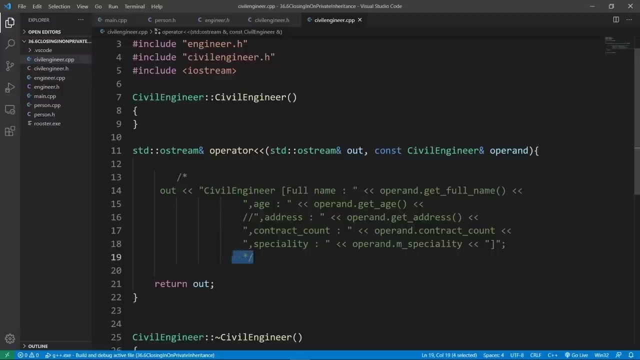 is not going to have direct access to these members because they are going to become private to this class here. and that's the experience we have if we try to use any of these methods and members we get from engineer, this is not going to work because they are now private to the engineer class. this 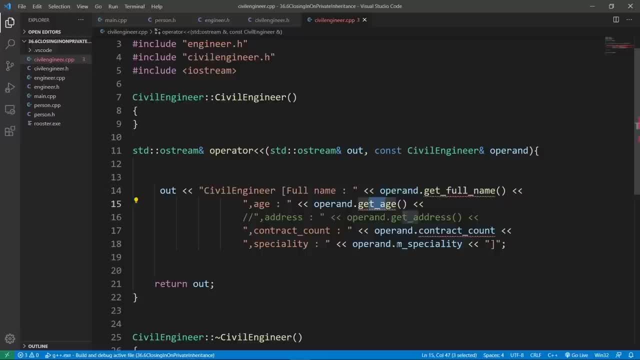 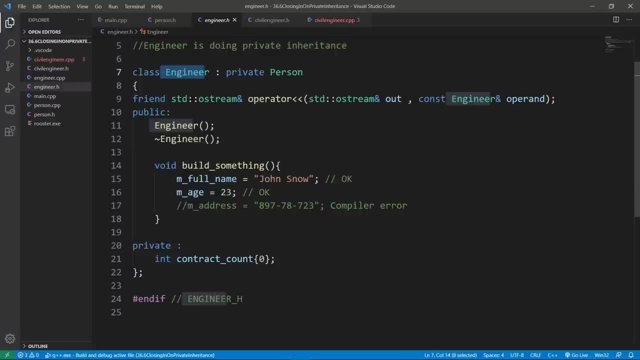 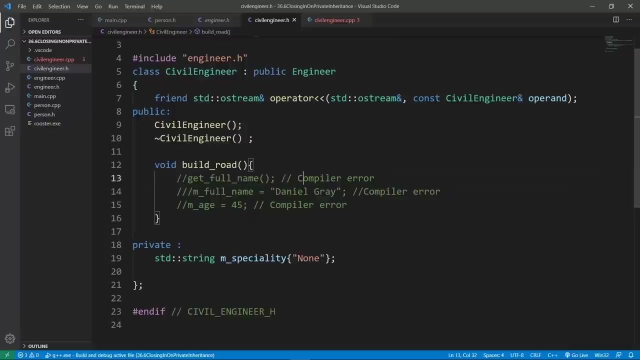 is the message here. so the get full name, get age methods are not going to work. if we try to use the contract count member which comes from the engineer class, that's not also going to work. if we look in our header and try to use any of these members, we're going to get compiler errors. 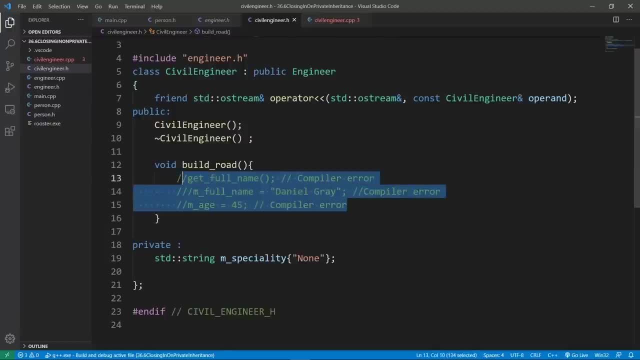 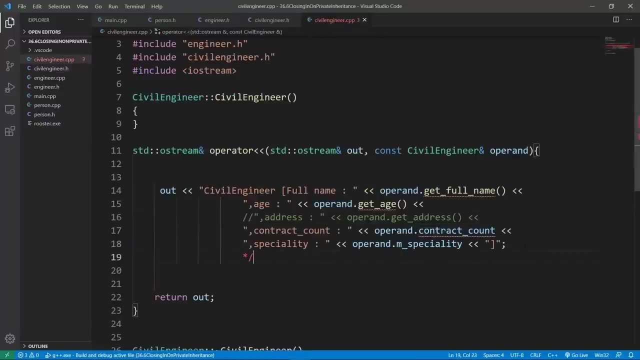 because all these guys are now private to the engineer class. this is really all i wanted to share in this lecture. let's head over to the cpp file and comment this out again, because i don't want to leave you with these compiler errors. i hope you found this lecture informative and fun. 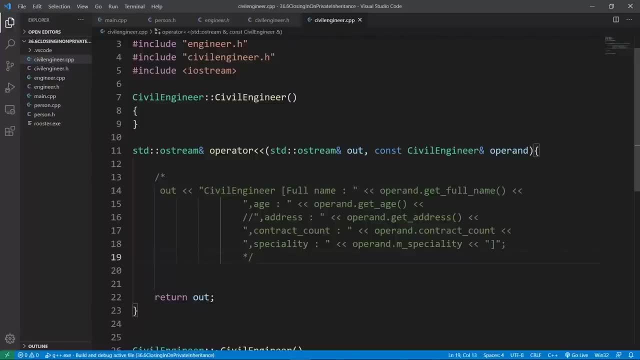 we are going to stop here. you this one. in the next one we're going to see that we can actually resurrect some members back in scope if they were eclipsed by the kind of inheritance we did from an upstream class. go ahead and finish up here and meet me there. in this lecture we're going to explore how we can. 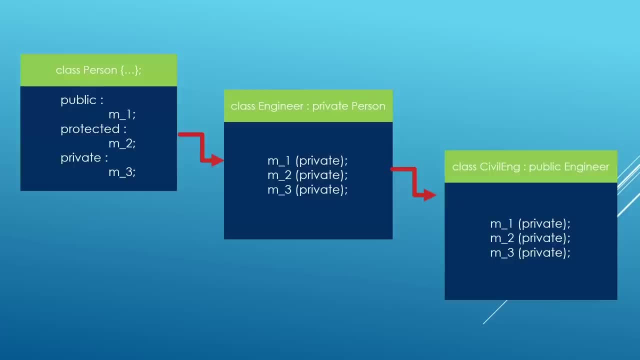 resurrect members back in scope. so what do we mean here? suppose we have our trusty inheritance tree. here we have a base class person. the engineer class is going to be the one that's going to do private inheritance- and it's going to really be selfish and say: i am going to take everything i. 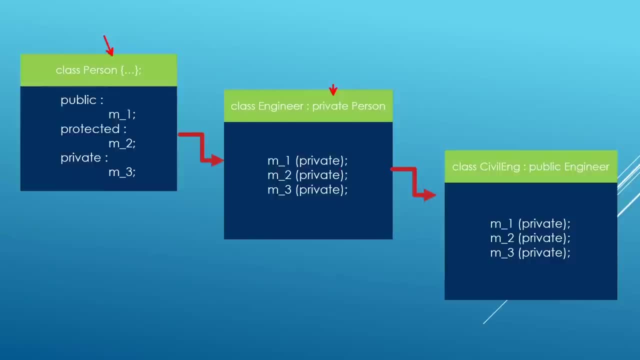 can from the upstream person class, but i am going to make everything my own and nobody inheriting from me will have access to these guys. for example, m1 and m2 are going to be private to the engineer class, starting here. when the engineer class does private inheritance, so any other class, for example, 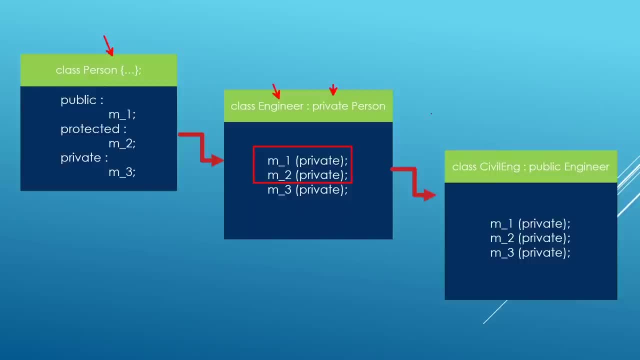 civil engineer, which is inherited from the engineer class in any way, won't have access to the m1 and m2 member variables. so suppose, for some reason that we have this kind of setup here, but again, we want some members to be accessible to other downstream classes. suppose, for example, 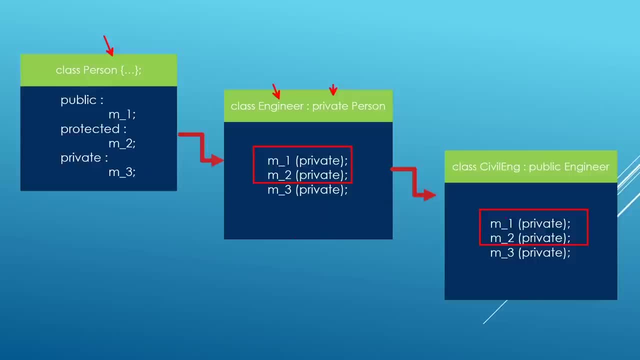 we want the m1 member variable to still be accessible to downstream classes, while we have done private inheritance. c plus plus is really weird in a way. it is going to work hard to really prevent you to do things and then give you a back door you can go through to. 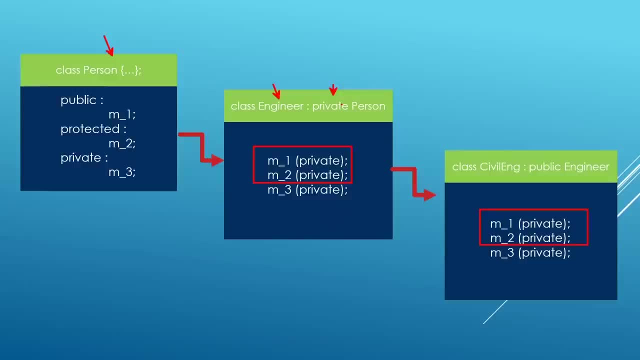 allow the same thing you are trying to avoid in the same place. it is the same kind of logic we have here: it allows you to use private inheritance to prevent downstream classes to access access to anything you got from upstream classes, but then again it allows you to change that and 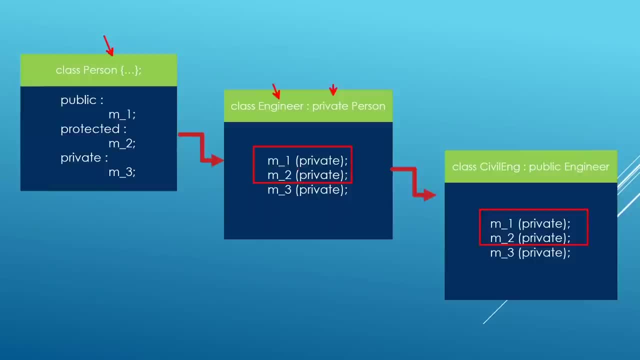 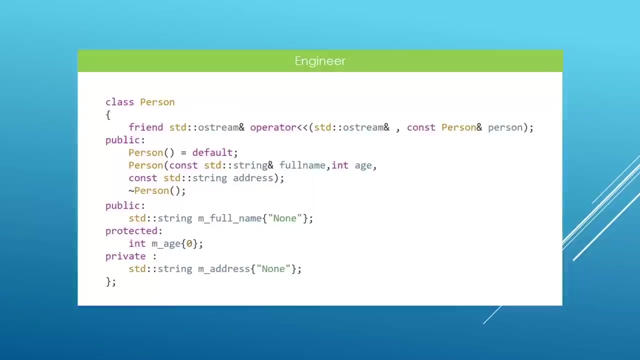 relax the access to downstream classes. for example, we can change the access of m1 and m2, make it more relaxed, make it public or protected if we wanted that. so let's take a look at some code, because I know that these things can really be confusing. okay, we are going to start from a person class. 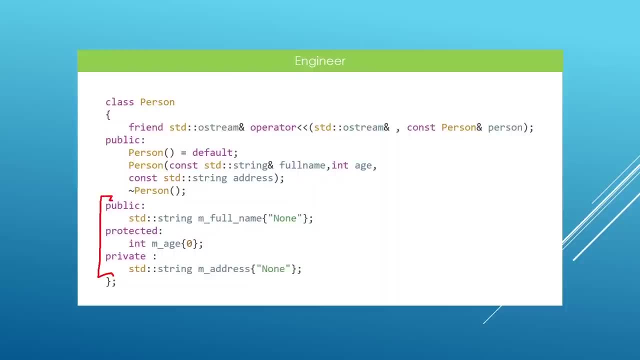 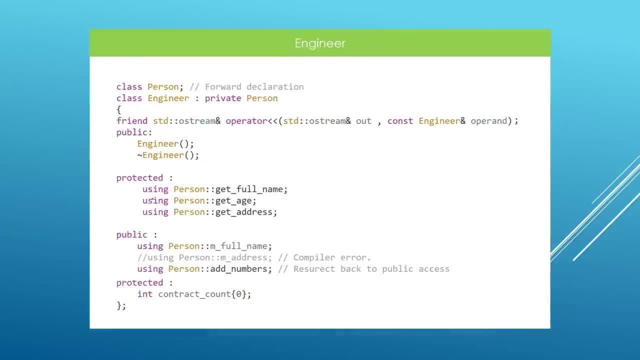 which is going to have a bunch of member variables. we will also have a bunch of gators that are going to return all these member variables and we are going to do private inheritance from person in an engineer class. this is going to strip down access to the members we get from person to private level. 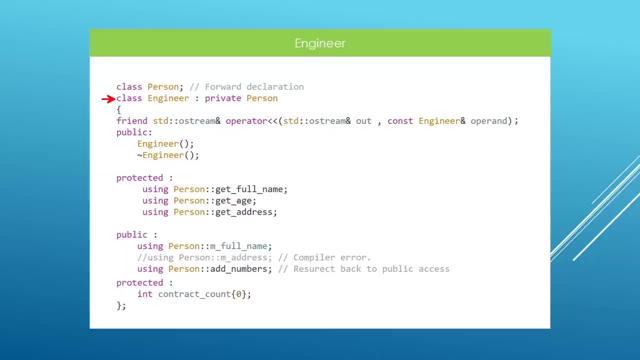 access, for example, the gate full name member function, the gate age, the gate address member functions are going to be private to the engineer class now, but for some reason you might want to resurrect them to a more relaxed access level. and you do that using the using keyword. so the first thing you need to do is to choose the section in 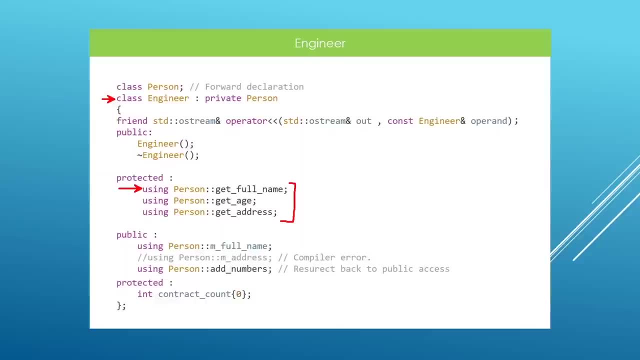 which you're going to be putting these, using statements, for example. because we put them in a protected section, all these guys are going to be resurrected with an access level of protected. if we put them in a public section, they are going to be resurrected with a public access level and they are going to be accessible from inheriting classes. one thing: 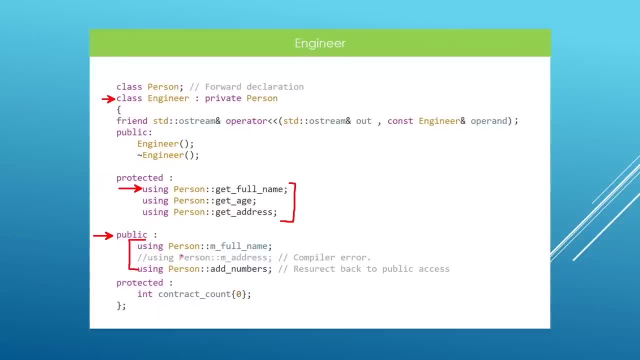 you should know is that you can't resurrect something that is already private to an upstream class. for example, we know that our M address member variable was private to the person class, so we can't really resurrect that in an inheriting class. if you do that, we're going to get a compiler. 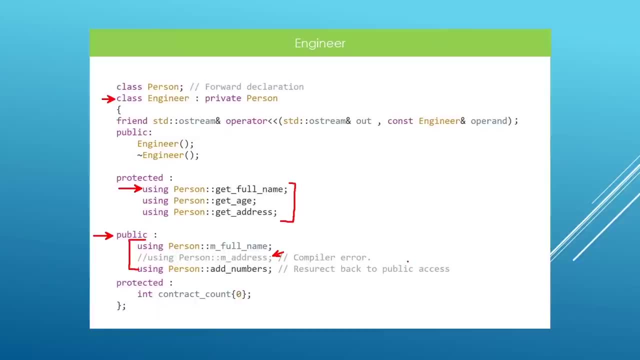 error and hopefully this is going to drive the point home that private inheritance is really really serious and that it's going to strip down access to private level access in an inheriting class and any downstream inheriting class will never be able to resurrect those member variables to a more relaxed access level. so because everything here is inherited as 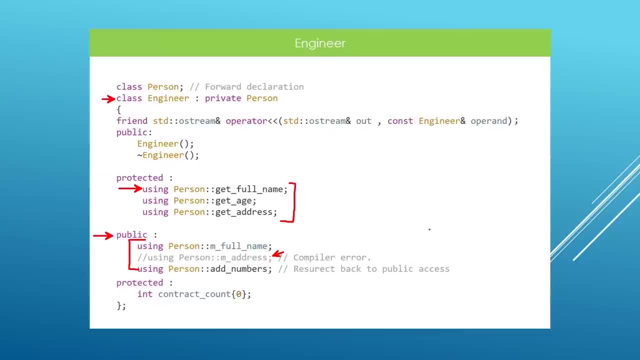 private by default. any downstream inheriting class will never be able to resurrect these guys, for example, to public or protected scope. this is the message here, and you can use this kind of design if you want that, but personally I don't like to do this because it's going to make your code much more hard to read and understand. if you, 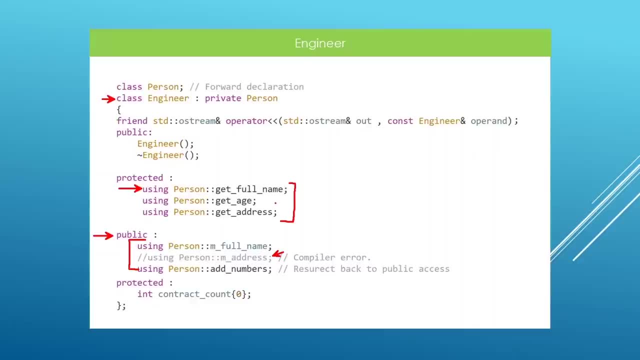 want these guys to be public or protected, why not make them public or protected in the first place and really not use private inheritance? that's going to be much more direct to see and understand and your code is going to be easier to work with for you in the future or for some other. 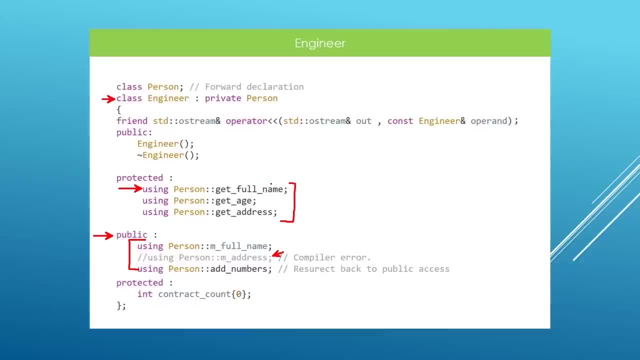 developers that will get to work on your code in the future. so this is the message here: you can use this feature to resurrect members back to a relaxed access level, and now that you have an idea about this, we're going to head over to Visual Studio code and play with us a little more. here we are. 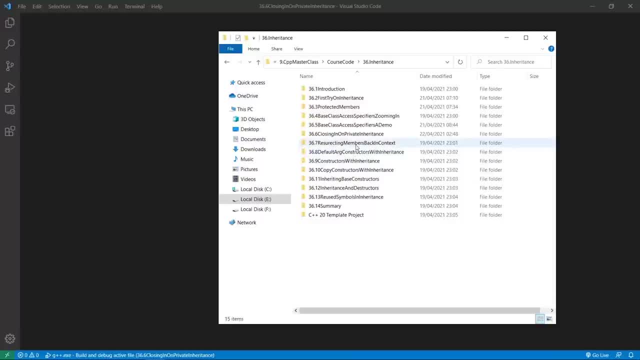 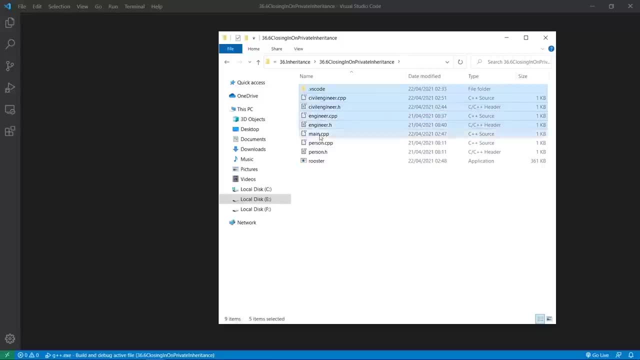 in our working folder. the current project is resurrecting members back in context. we are going to completely reuse the code from the last lecture because it's going to give us a new starting point. we can copy everything except for the binary here. we don't need that in our 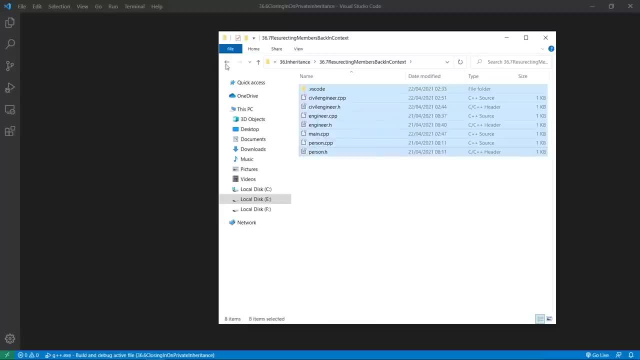 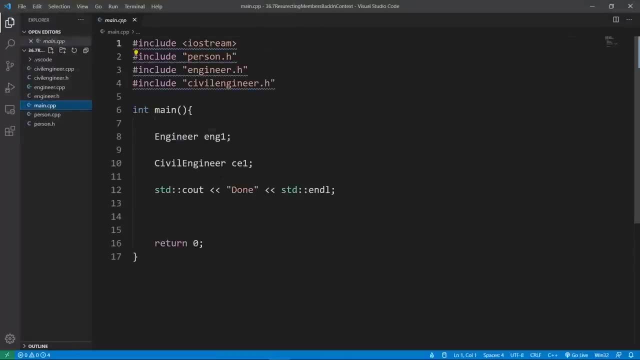 current project. we're going to put in our starter code and we're going to open this little guy in Visual Studio code. so we're going to have our code, we're going to have our main function and we're going to have all these objects created here. I'm really not sure if we're going to need this yet. so 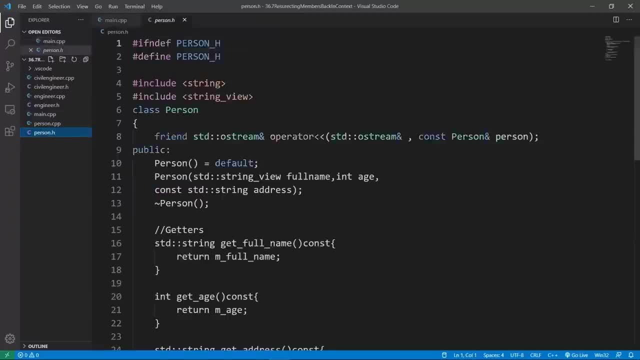 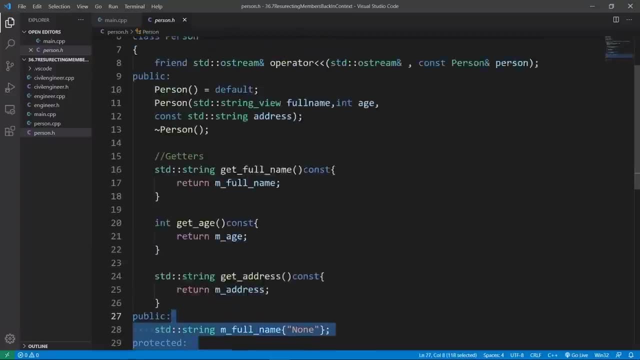 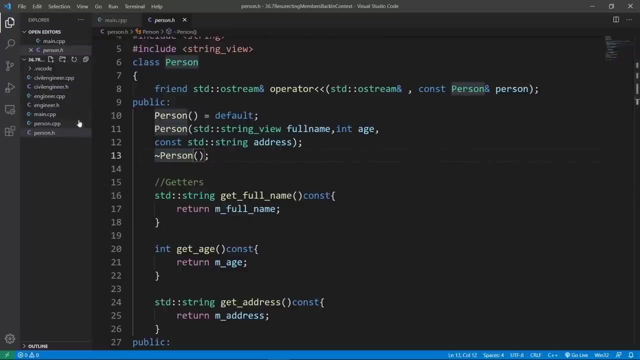 let's take this out and we're going to look at our person class. it is going to have our members here and we are going to have a bunch of getters which are going to be returning these member variables and we have a constructor here which is really going to build a person object. nothing complicated here we have an. 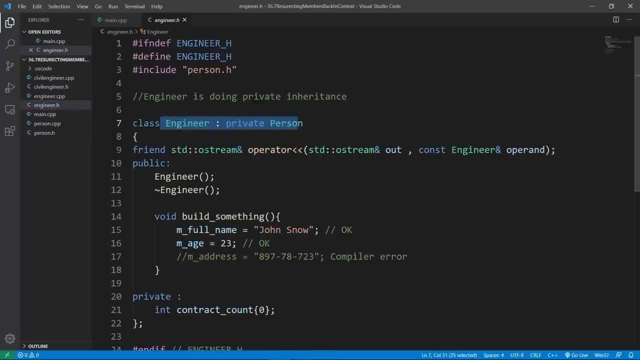 engineer class which is going to privately inherit from person and we know that this is going to Eclipse everything that is not private in the person class to private level access. so everything is going to be private to the engineer class now, but sometimes we don't want to. 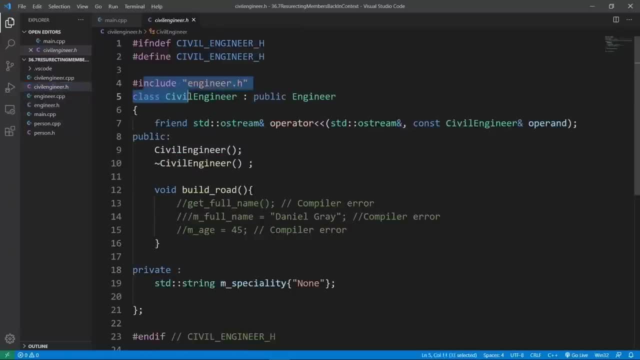 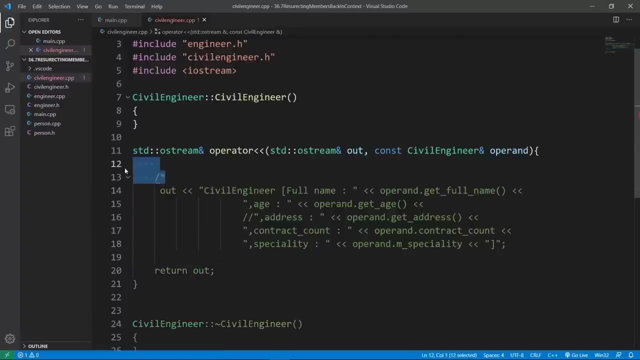 do that. for example, if we go down in our civil engineer class, we're going to see that the gate full name and get age methods are going to be private to the upstream engineer class and that's going to break the code for our output stream operator and it's not going to work because we won't have access to. 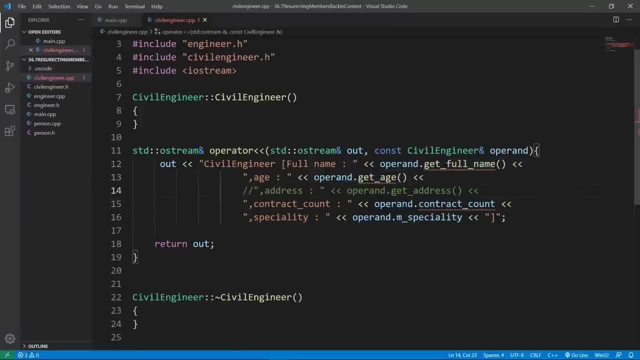 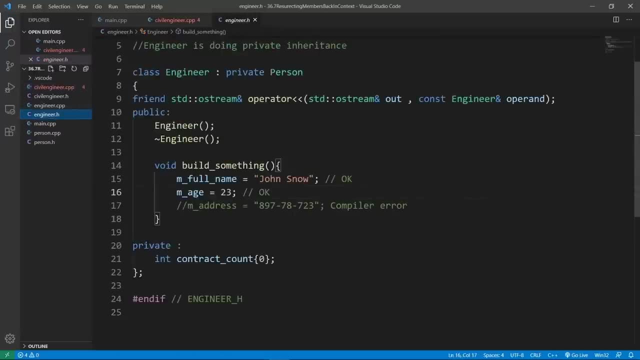 get full name and get age and that's also going to kill access. we had on the get address method, which would give us access to the address member that we have in our person class. let's make sure we are looking at person. I am confused here. we. 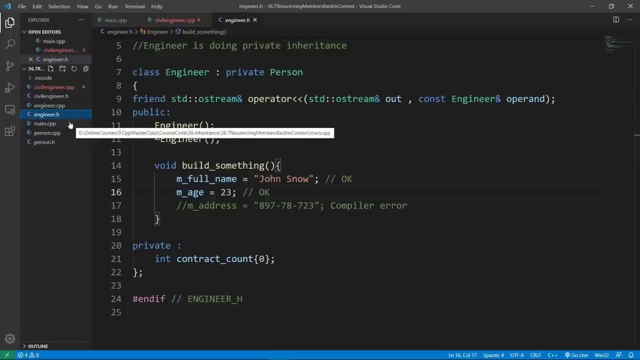 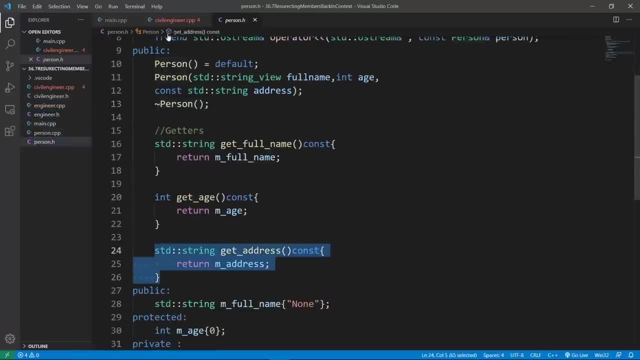 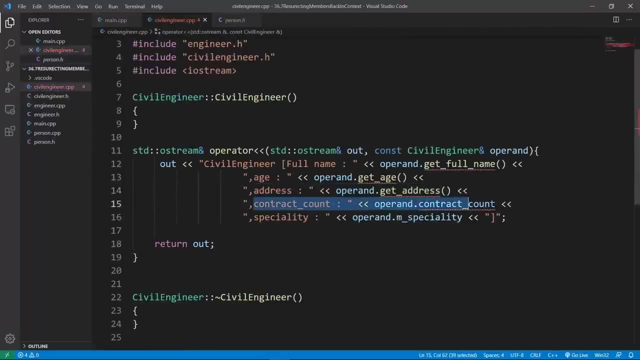 have a lot of pieces of code here. where is the person header? it is down here. so we have the get address method, which is going to return the address. we want to have access to that in our civil engineer class to be able to print all this information if we also want to print the contract. 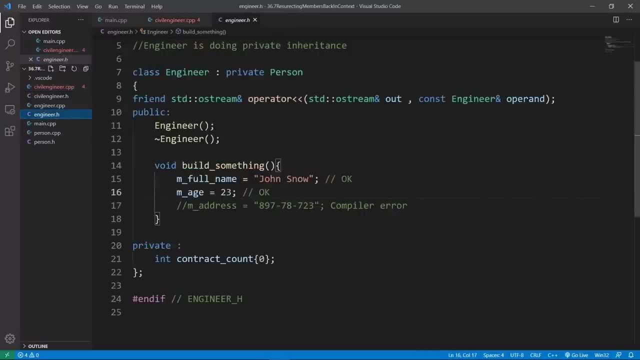 account. we can go in our engineer class and put in a method which is going to return that, so we can say end and say get contract count, and this is going to be a constant member function because it's not going to be modifying our object. we're just going to return a value, we're going to return a contract account and we can go in. 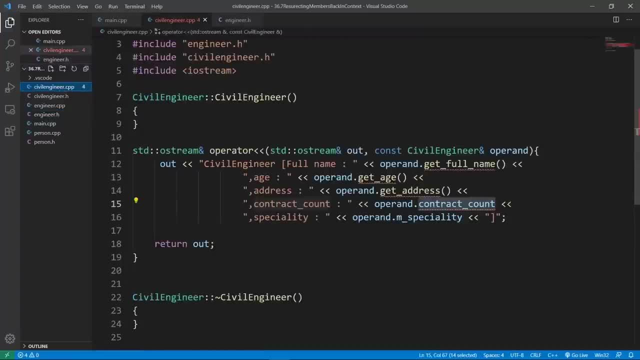 our civil engineer implementation file and change this to say: operand get contract account. we can do that. okay, we have this method. now we want this to work. this is going to work because we are doing public inheritance from the civil engineer class, but we want this to work. we. 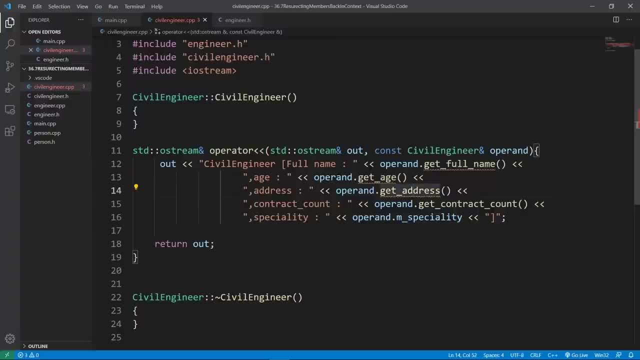 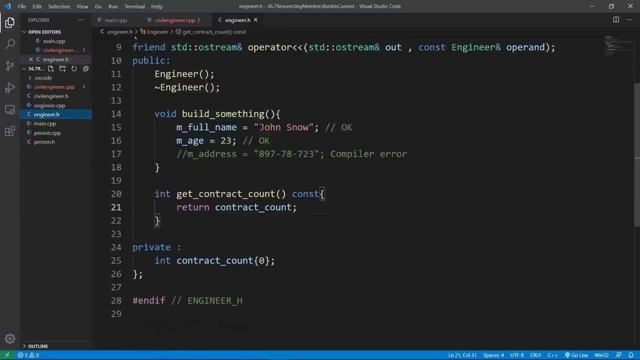 want to get full name, get age and get address to work here and we can use the using feature to resurrect these members to an access level which will allow our civil engineer class to pick them up so we can go in our engineer class and set up, for example, a public or protected scope. we're 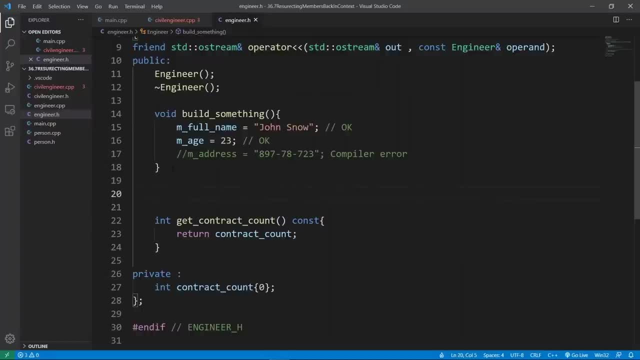 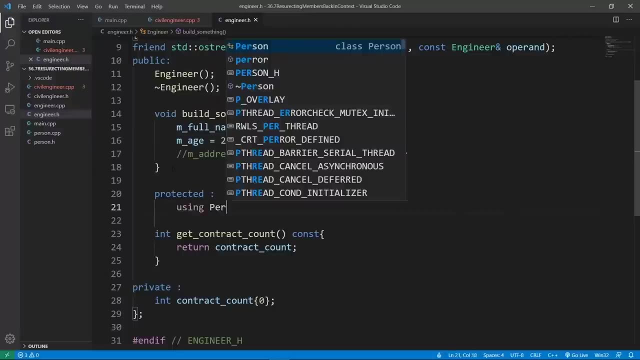 going to use protected, because we want these to only be accessible um inherited classes, for example. so we're going to say protected and we're going to say using. this is the syntax. we're going to say person and we're going to say get full name. we're going to say using 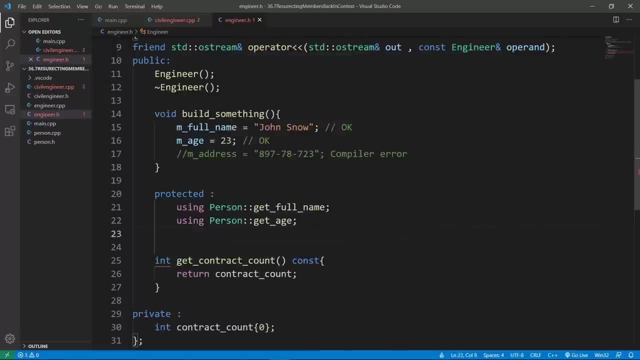 person get age. we're going to choose this and we are going to say using person and say get address. I think we have that method here. the moment we do this, we're going to go in our civil engineer class. you're going to see that it is going to work now, because what we just did is resurrect this. 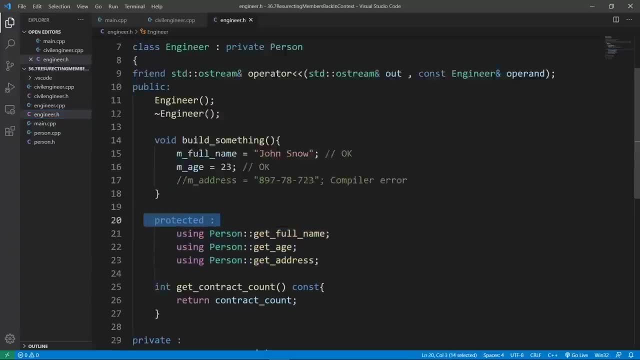 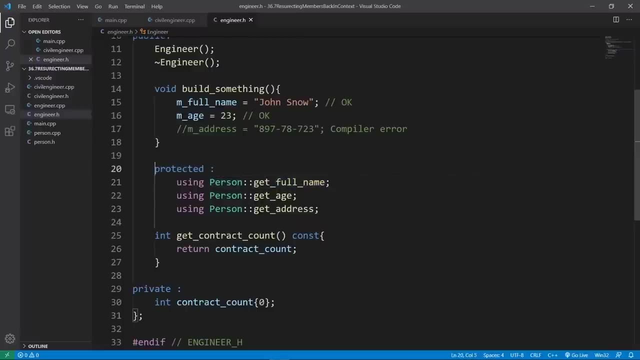 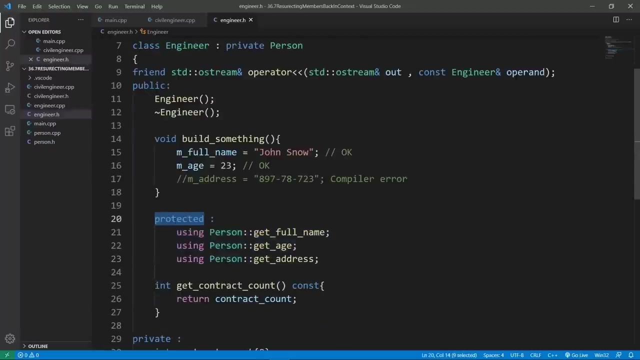 members to have protected access level in the engineer class. so the inheriting classes are going to look at this and see that they have a protected access level in the engineer class and they are going to be forwarded down to any inheriting class. we could also change this. 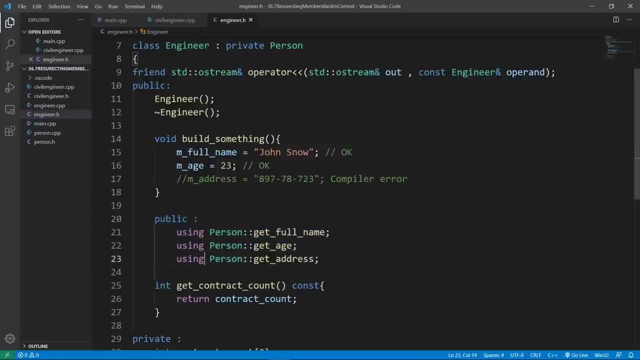 to public. this is also going to work. they are going to be inherited as public and hopefully you can see that any member that you resurrect it's going to take the access level of the section here you resurrected. if we resurrected them in a public scope, they are going to be resurrected. 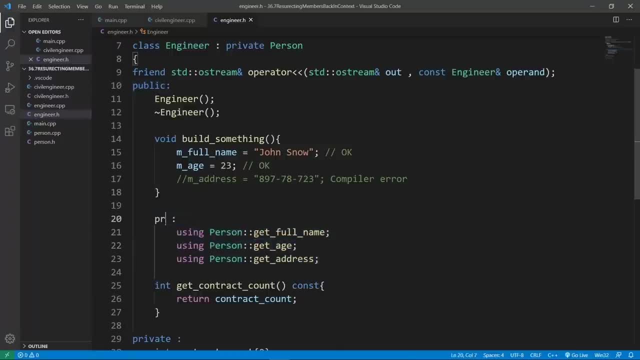 with a public access level. if we resurrect them in a protected scope, they are going to be resurrected with protected access level, and this is the message here. now, if you happen to have a bunch of overloads in an upstream class- for example, suppose we have a bunch of add functions in the personal 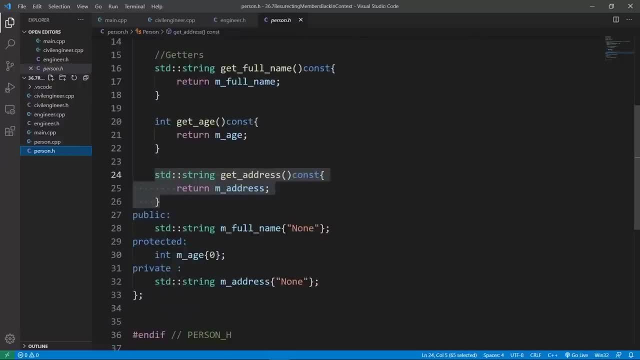 class. we can go in and put in, let's do that. we can go down and say double or end, let's say end. so that's going to be much simpler. we can say add and say end a, and say end B and say end C. we're going to. 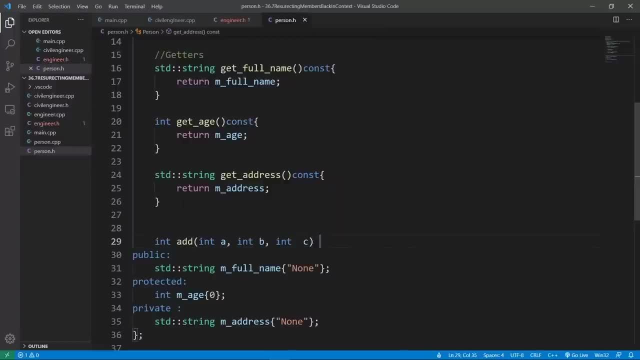 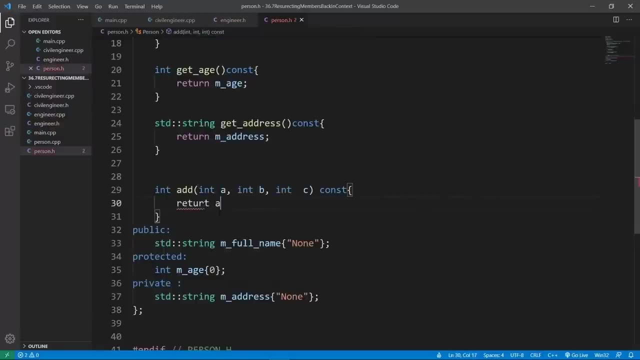 have three things that we are adding. this is going to be a constant member function. it's not going to be modifying our members in any way. so we're going to return a plus B plus C- this is something we can return from a member function here- and we're going to do an overload of the add member to do. 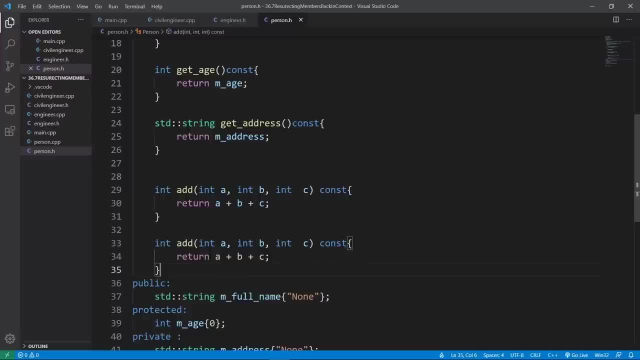 the addition of two parameters. so we're going to only have A and B and I think we can use A and B in the first overload here. that's going to be much easier to follow. so we have one that adds two parameters and we have another one which is going to add three parameters. if we privately 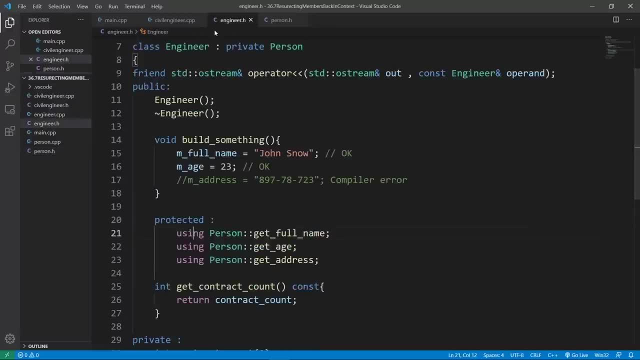 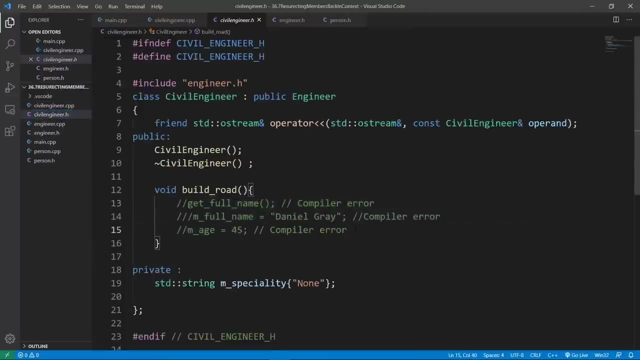 inherit from person. these guys are going to be stripped down to private level access in the engineer class and they won't be accessible from in any other downstream class. so, for example, if we head over in our civil engineer class and trying to say, add 10 to 2, for example, we're going to get a compiler. 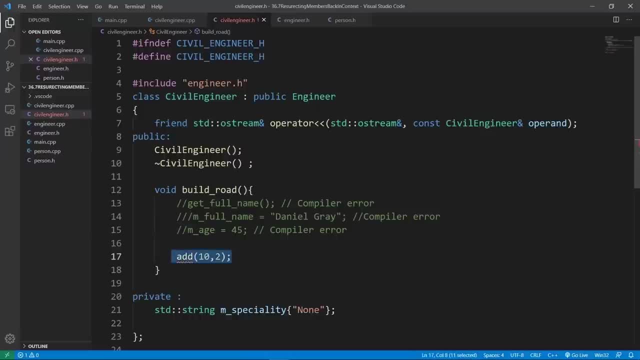 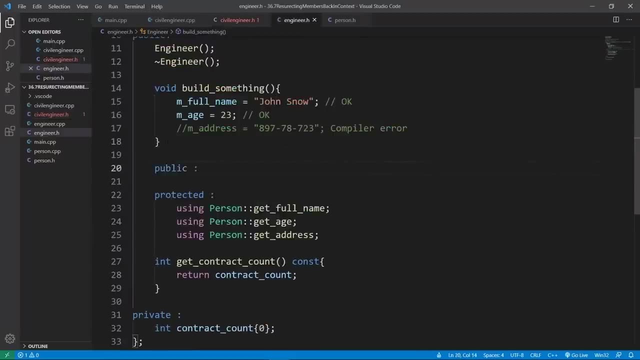 error because we don't have access to this. but we can also resurrect these add members in our engineer class. so let's go there and we're going to set up a public section in this class here and we're going to say, using person add, this is going. 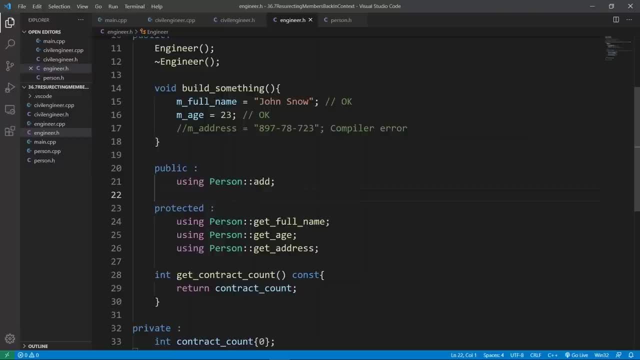 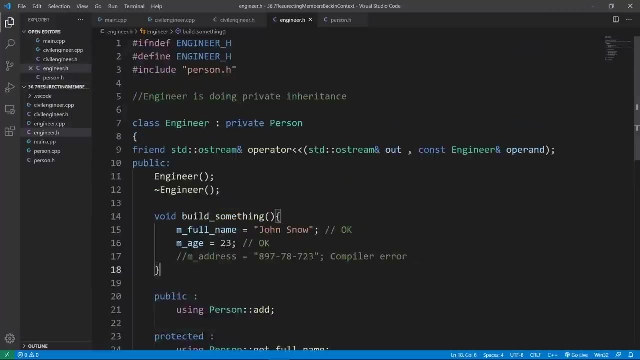 to resurrect all the overloads that we have in our upstream class. and this is going to be the case because we resurrect only based on the name of the function, and the same name for a member function can be shared by many overloads. so if we do this kind of resurrecting, we are doing for the 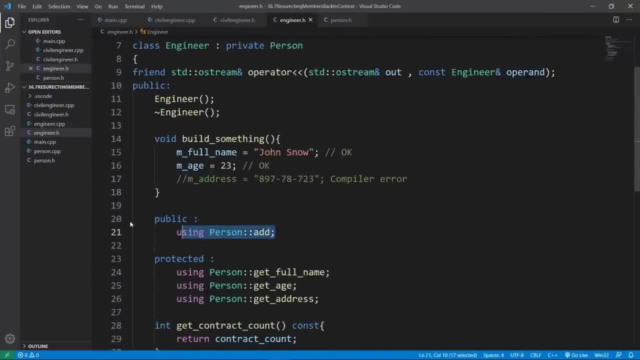 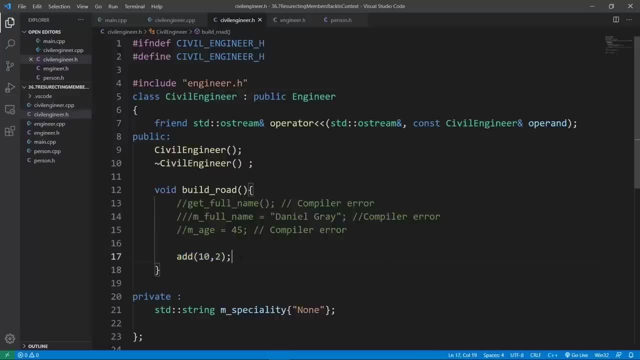 add member function from person. we are going to get all the overloads if we go in civil engineer. we will be able to use the member function taking two parameters. we will also be able to use the one that takes three parameters. they are all going to be resurrected here. this is the message I want. 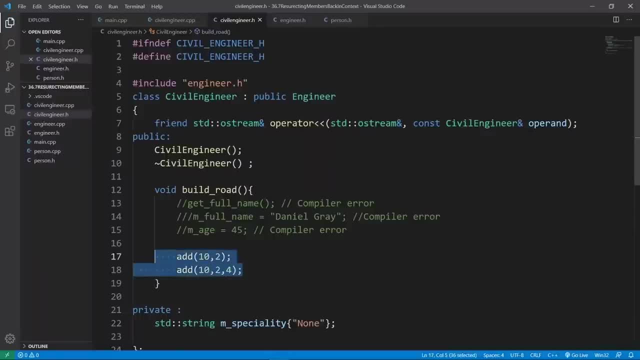 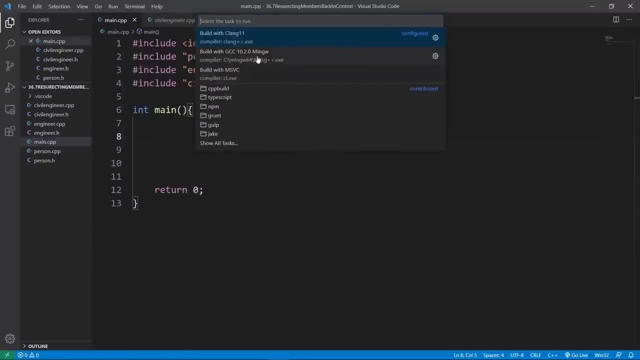 to convey. if we do this, you're going to see that this is going to work and our code is going to just world. fine, let's world and see if the world is good. actually, we're going to pass this through. the world is going to be good. so everything is working just fine and the message I really wanted. 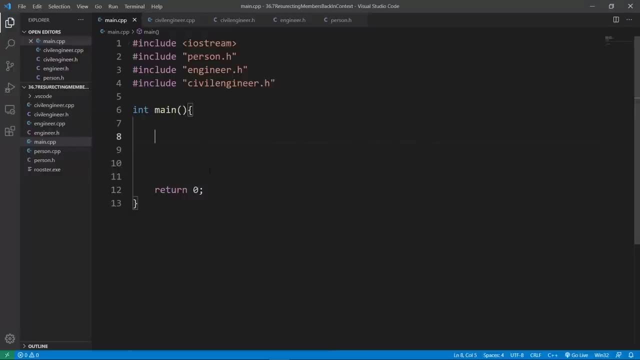 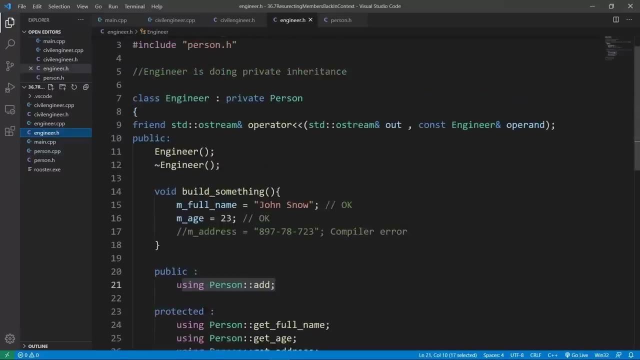 to convey is that it is possible to resurrect members in a more resurrected access level if you are inheriting using a really constrained base class access specifier. for example, we are inheriting using a private access specifier. this is going to Eclipse everything we get from the 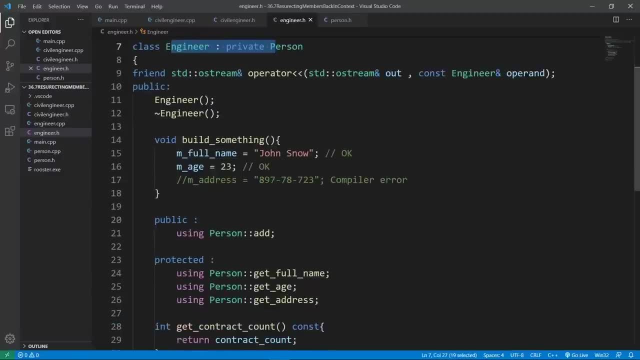 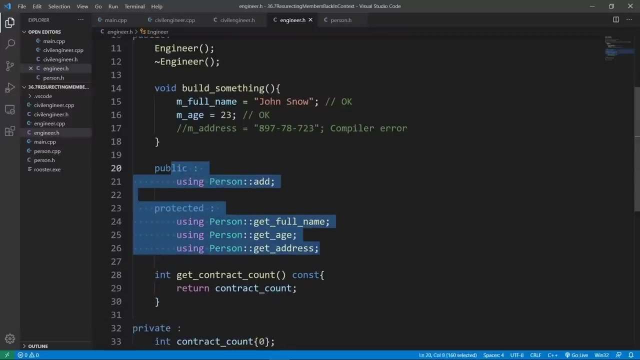 upstream class to private level but think that's too much and you have a few members that you would like to put in a more relaxed access level, you can use this resurrecting feature and it is going to make things accessible in downstream classes if that's what you want in your program, and again i hope this drives the point home that 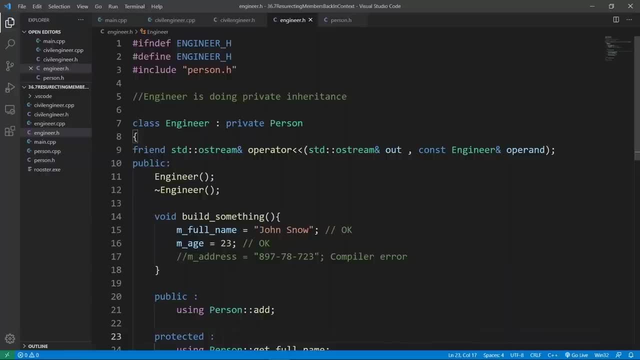 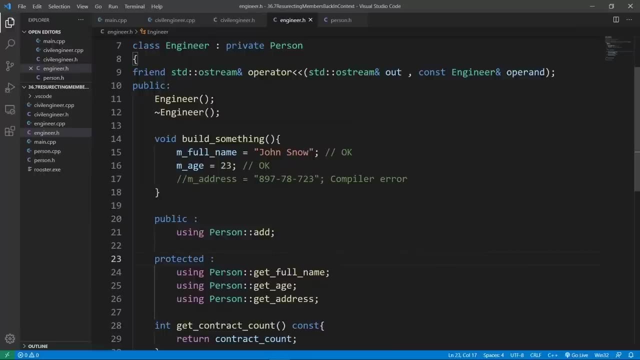 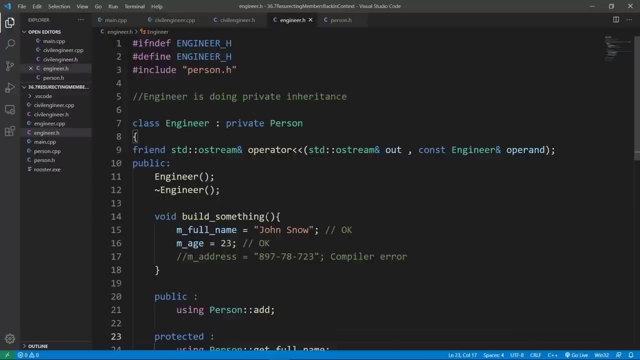 c++ is going to sometimes work really hard to prevent you from doing one thing and then again give you a back door you can go through to do that same thing. this is the same thing here we are doing private inheritance, but we are allowed to kill or relax the effects of private. 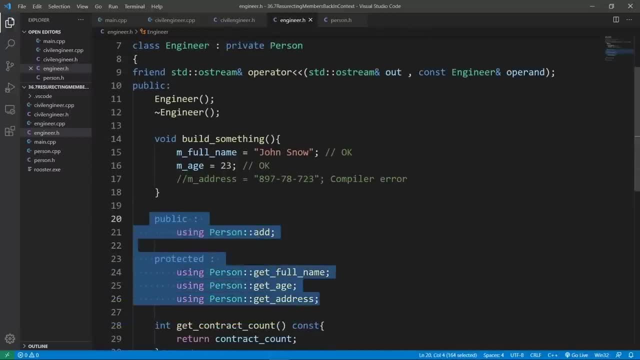 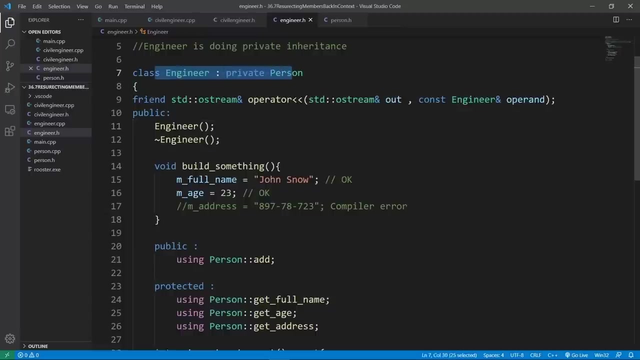 inheritance by bringing things in a more relaxed access level, and you can use this if it makes sense for your code. again, i don't like this personally because it's going to make code confusing. if other developers see that you are doing private inheritance, they are going to expect everything from the upstream class to be private to the class that is doing. 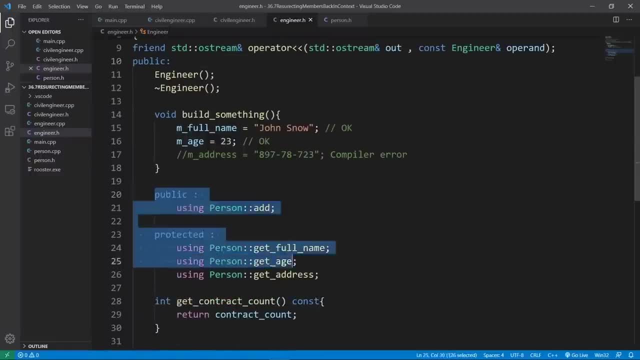 private inheritance and if they see that they can use these things that should be private by default in downstream classes. this is really going to confuse them and it is going to cost them more minutes to look at your code to really understand what is going on. so if you really want these things, 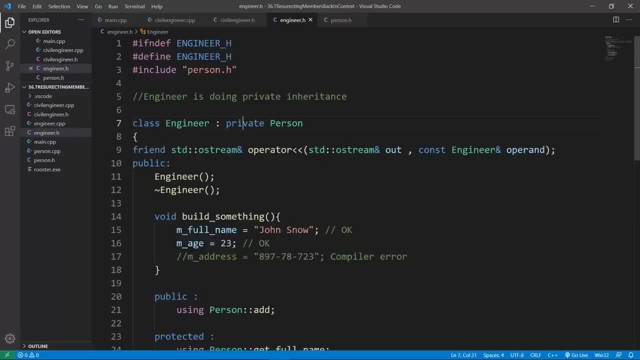 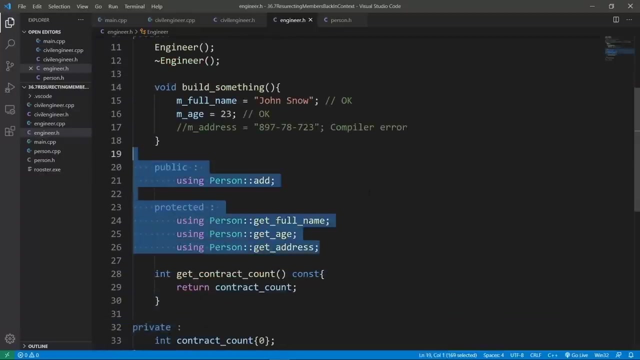 to be accessible in downstream classes. why not do public or protected inheritance in the first place? this is my argument here, but it is going to be your choice. my job here is to make you aware of the possibilities that you have in the c plus plus programming language. okay, the last thing i want. 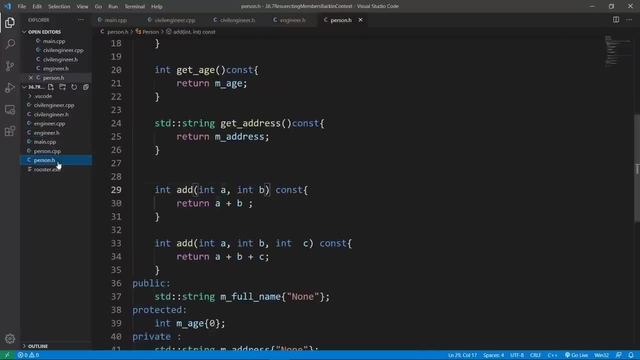 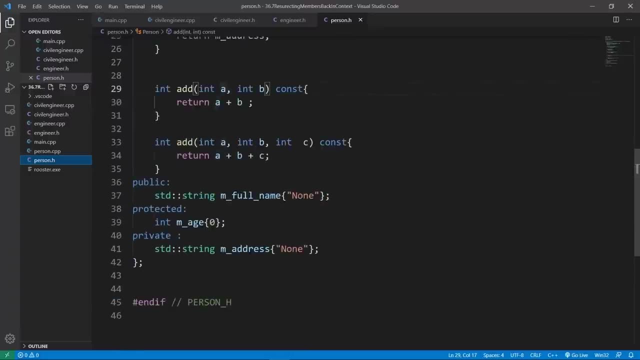 you to see in this lecture is that if there is something that was already private in an upstream class, you can't resurrect that. if you try to do that, you're going to get a compiler error. this is also going to drive the point home that you can also resurrect member variables. so far what we 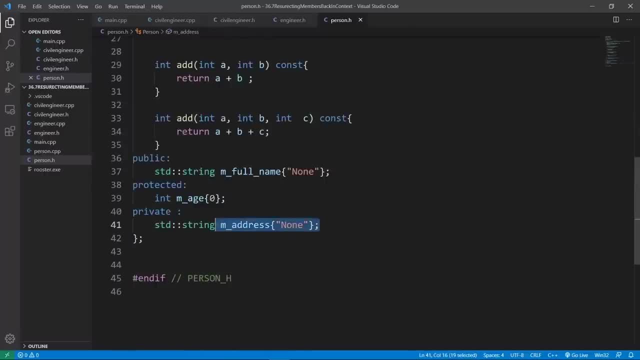 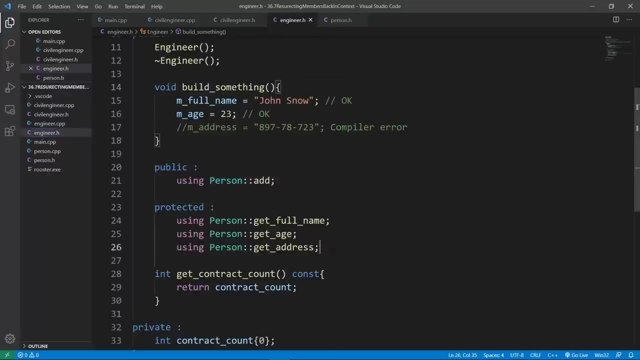 are going to do is we are going to try and resurrect all member functions and we can also resurrect member variables. so we're going to try and resurrect the m address member in the engineer class and let's see how this works out. so let's go in our engineer class, we can go in our protected. 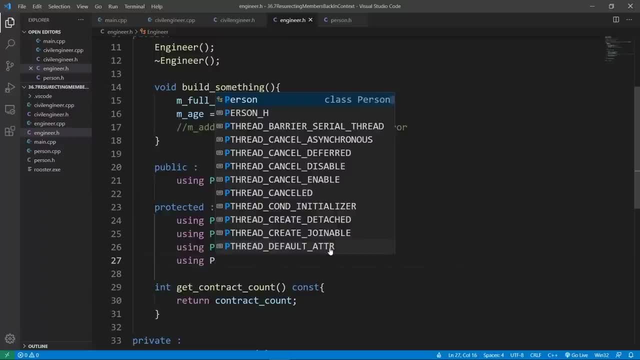 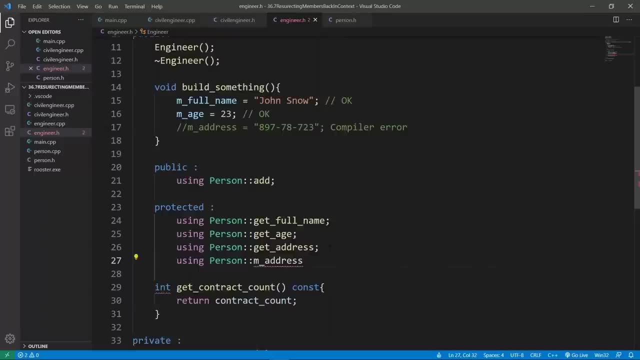 section. we can do this really in any kind of section. we're going to say user and we're going to say person and we're going to say m address. you see that this is not going to be, this is going to be assigned, that this is going to give us a compiler error, and if we're trying, 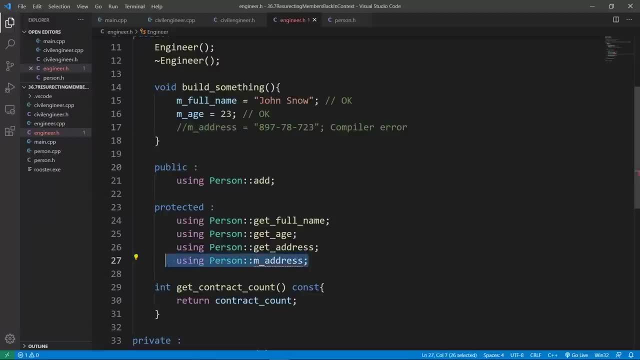 to do that. we're going to see that we're going to get a compiler error. the message here is that if something is already private in a nap stream class, you can't resurrect it. it is eclipsed down forever and hopefully this drives the point home again that private inheritance is really serious. 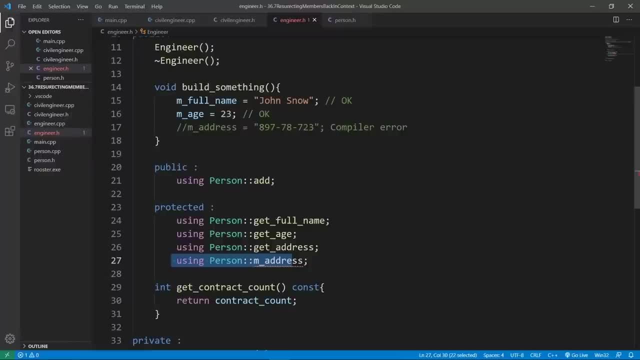 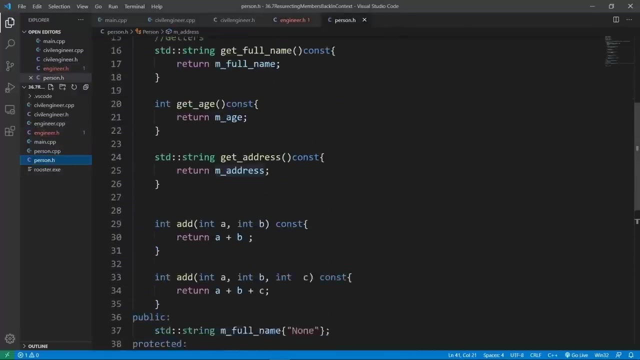 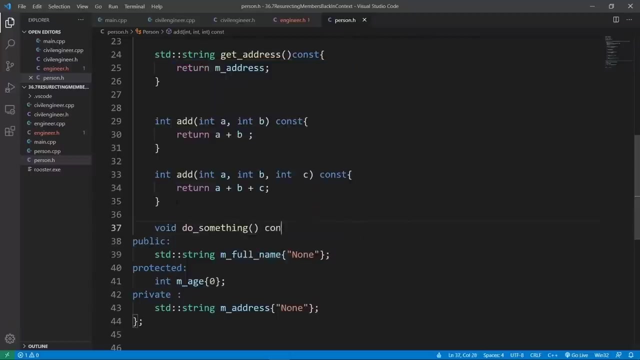 for example, in our civil engineer class we can't resurrect something that was already eclipsed to private level access by the engineer class. let's go in our personal class and see if we have any other member function we can uh play with. we're going to put in a member function that says do something. we're going to say, void, do something, and it's. 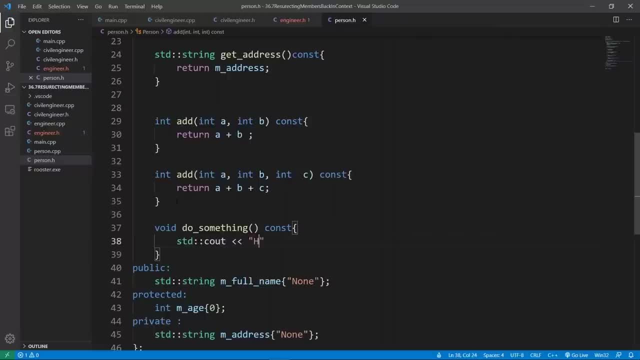 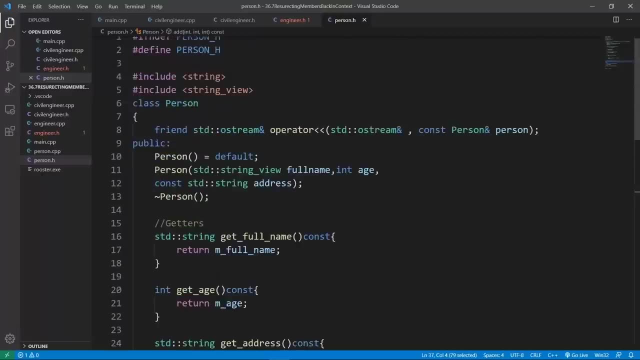 going to be cost. it's just going to say: hello, you can do something like this. we are learning and this method is going to be eclipsed down into private level access are doing private inheritance from person. let's go back in our engineer and comment this out. 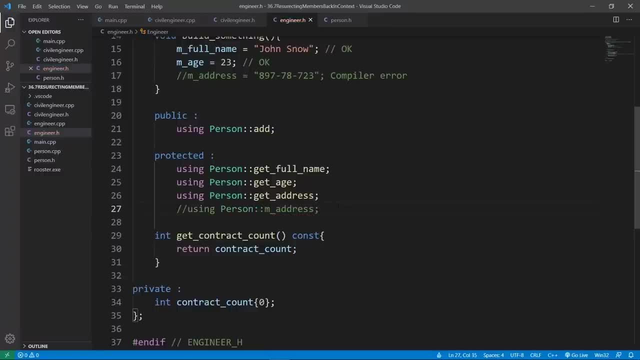 because it is going to give you a compiler error. if you build, you're going to get a weird compiler error. i think i should really show you this because we are learning here. so we're going to try and build our program anyway, we're going to pass this through gcc and we're going to see the 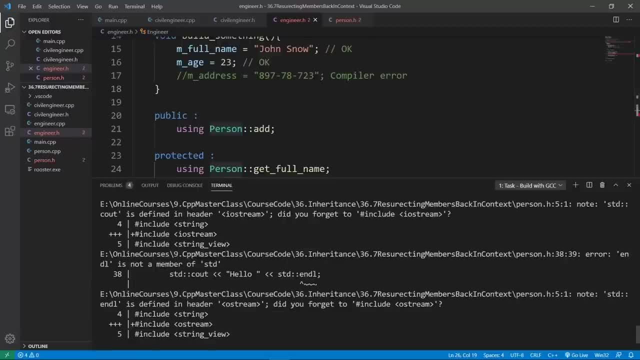 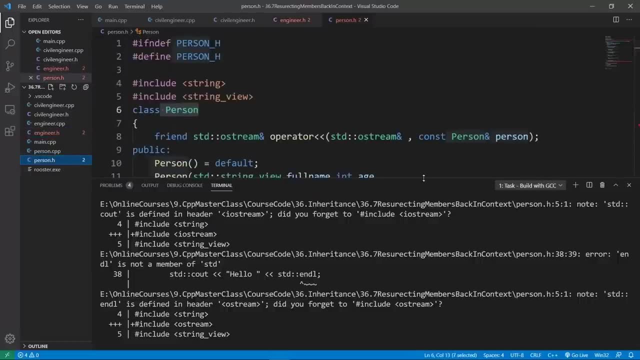 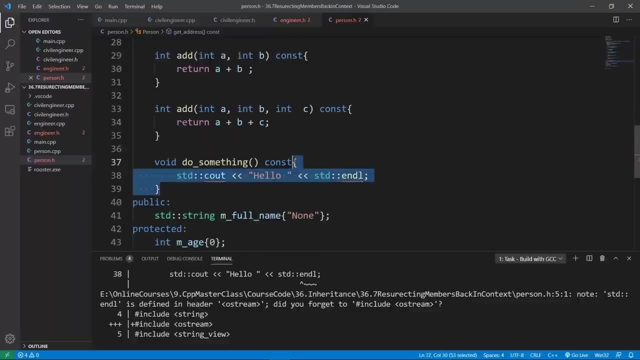 kind of compiler error we get and we are going to see that there's no member std. this is a problem we just introduced in our class here. i think to solve this problem we can just put our definition in the cpp file. we can do that. we're going to grab this and we're going to put the definition. 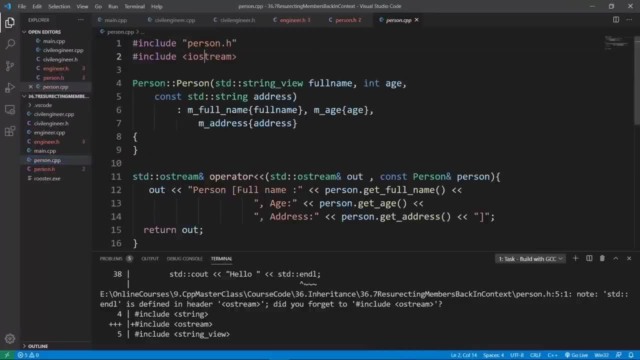 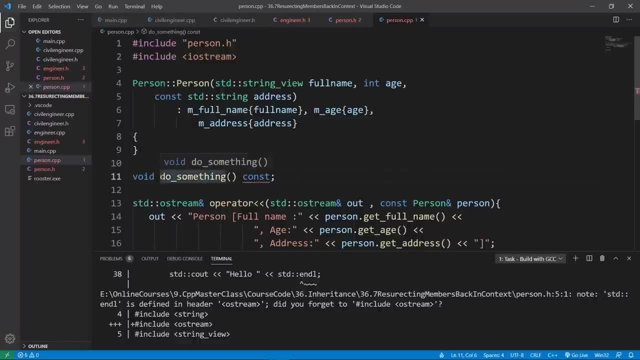 in personcpp, because we have io stream included in there. this is going to make our code work much better. let's do this. we're going to say void and say person and we're going to say stdc out, hello. this is going to fix you problem here, and the only problem we will have will be in engineer, where we are trying to access. 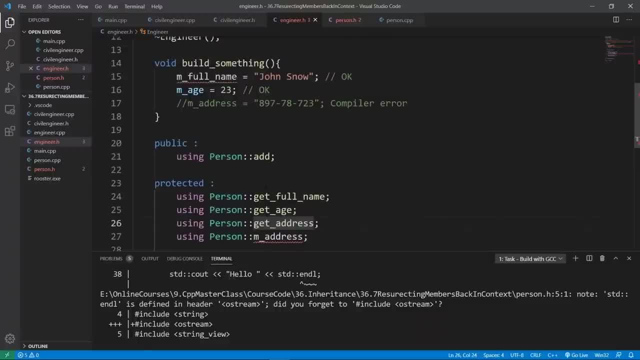 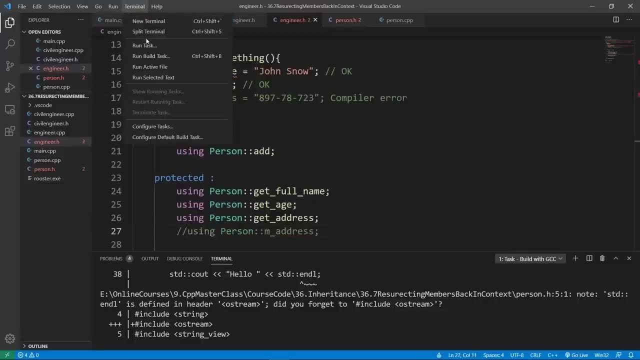 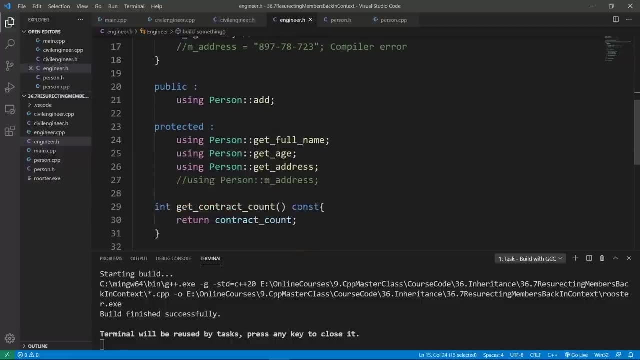 things that are now private to the base class. why do we have this squiggly line here? let's take out this and try to build, really make sure that this problem is not existent and it was visual studio code messing with us. so we're going to bring this in and build and we're going to see the kind of 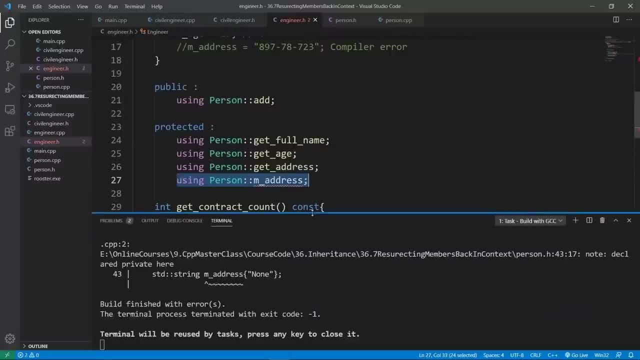 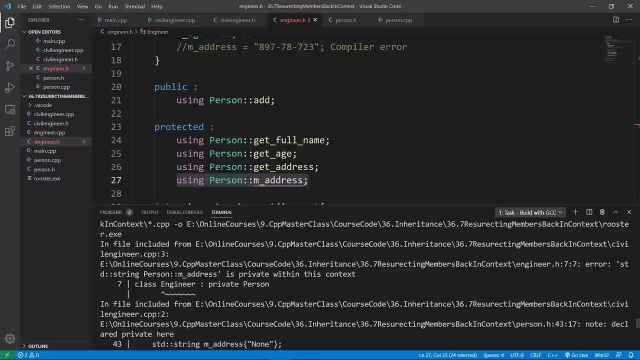 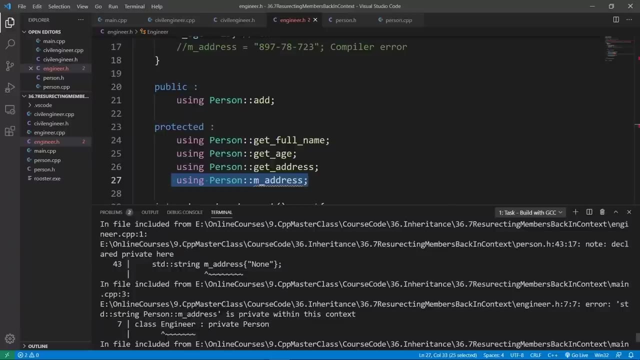 compiler error we get here. this is what i am trying to make, you see. you see, the build is finished with errors. if we go back, we're going to see that string person m address is private within this context. we can't really resurrect it. if we do this, we're going to get this compiler error here. this is the message. 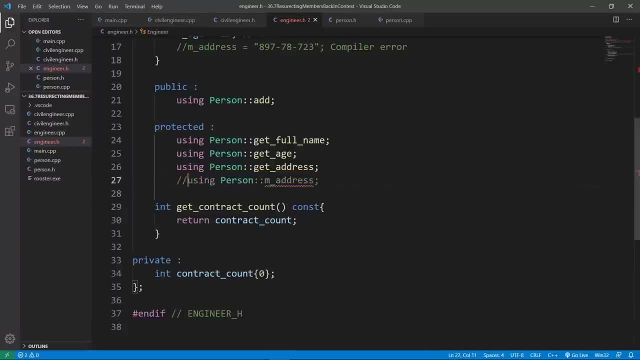 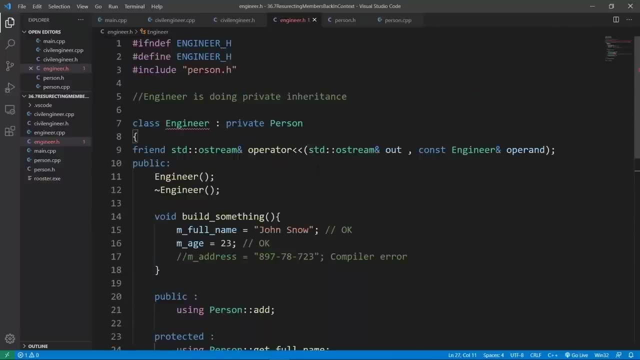 you shouldn't really try to resurrect something that is already private to an upstream class, and that's what we are doing here. we are trying to resurrect a member which is private to person, and this is not allowed in c plus plus. if we do that, we're going to get a compiler. 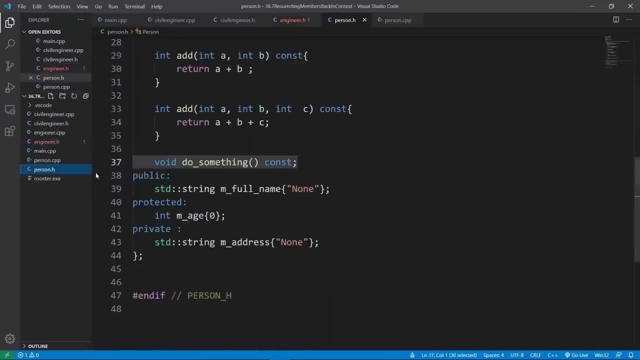 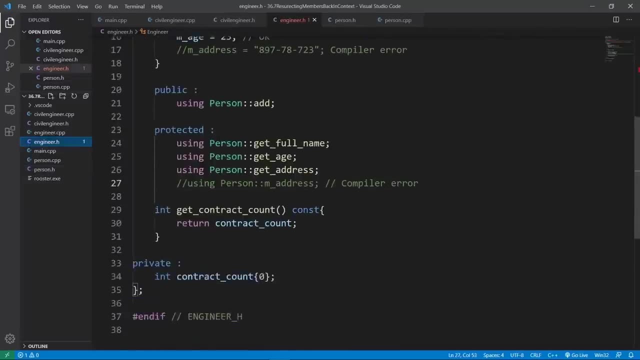 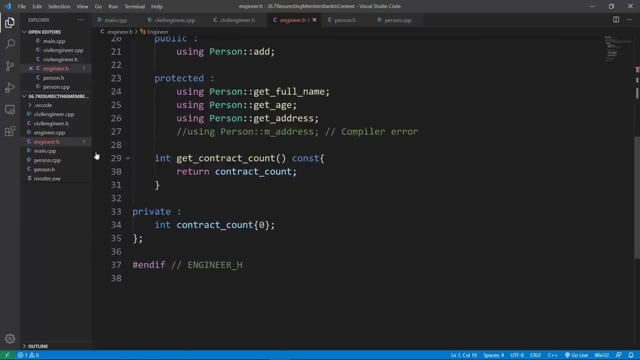 error. okay so, but what i want you to see here is that a public member which was in the base class was also a clips down to private level access in engineer. so if we try and resurrect the do something method in our civil engineer class, we're going to get 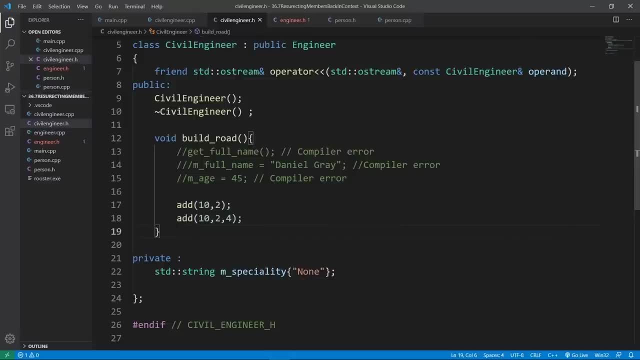 a compiler error. so let's try and do that. we're going to put a public section- why not? and we're going to go down and say using person and say: do something. we have this method here. but if we do this we're going to get a compiler error. 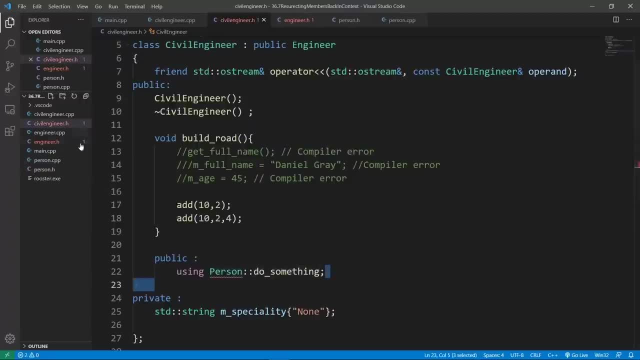 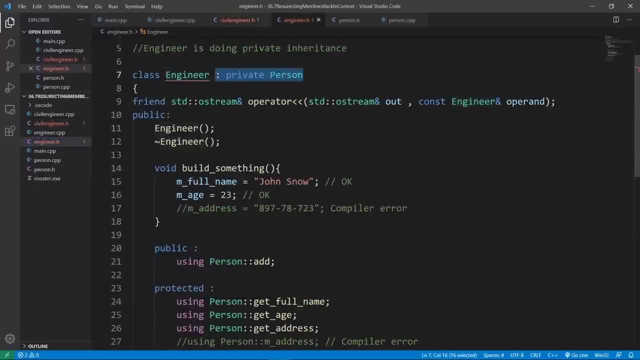 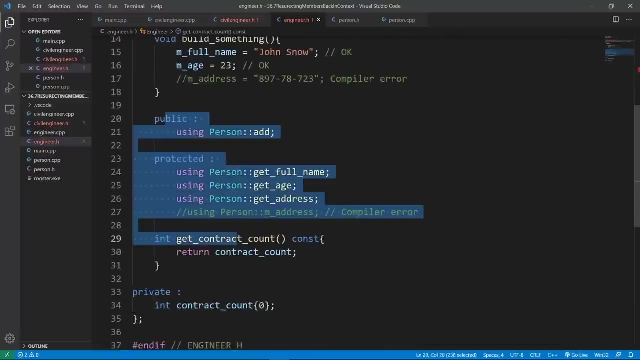 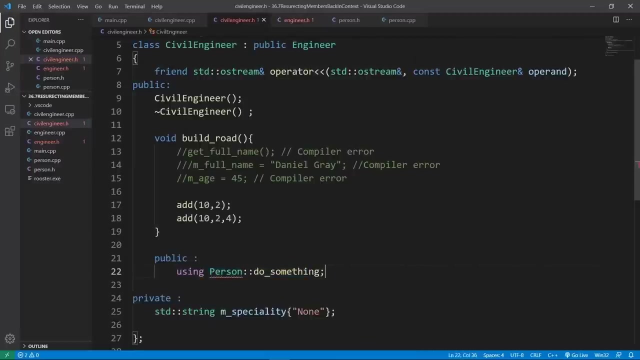 because this method is now private to the engineer class. and why is it private to engineer? well, engineer is doing private inheritance that's going to eclipse everything to private level access by default. so this member is private to engineer. we are inheriting from engineer in civil engineer and this is going to be already private to engineer and we can't resurrect. 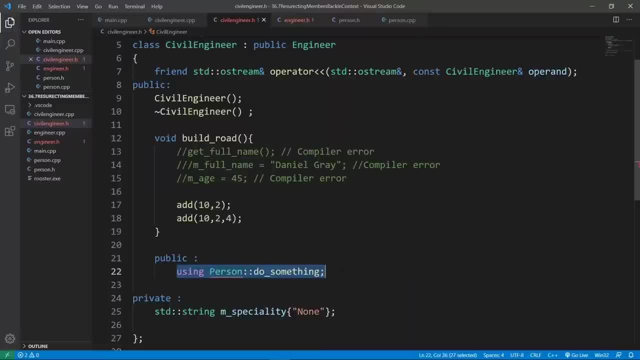 this back. so if you eclipse something using private inheritance, you want to be able to resurrect that to a more relaxed access level in downstream classes. this is the message i am trying to convey here. so this is also going to give us a compiler error, and if we're trying to build our 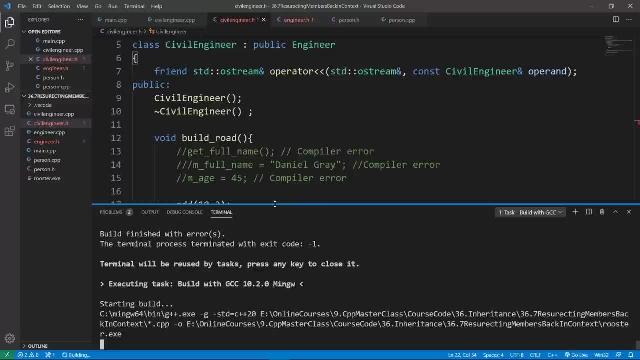 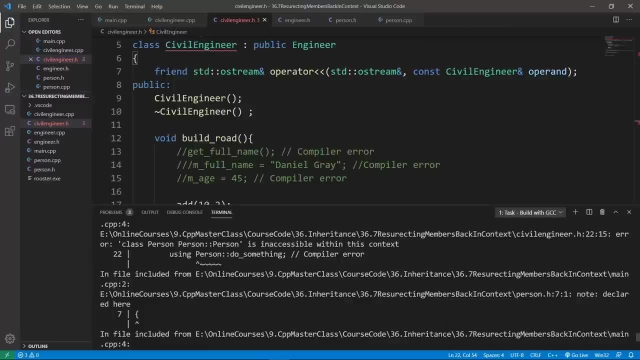 program. we're going to see that let's pass this through gcc. we are going to see: that's the world finished with errors? and if we go back, we are going to get some kind of error that says that do something is private to some class. it isn't accessible within this context. this is the message. 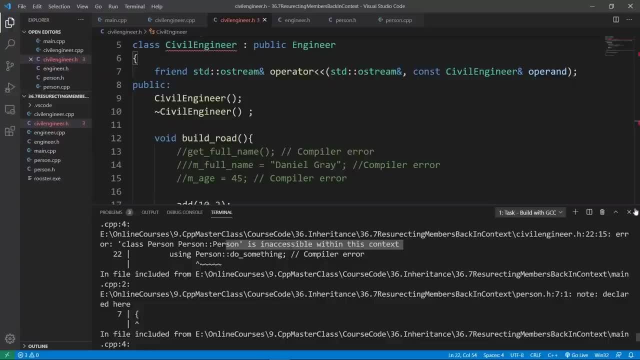 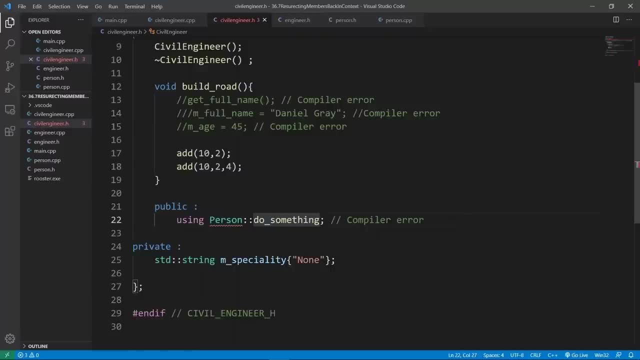 we get from this particular compiler we are using, but the bottom line is that you shouldn't really try to resurrect something that is already private to an upstream class, and this is what we are doing here. you shouldn't really do that. let's comment this out and get a code to compile again. 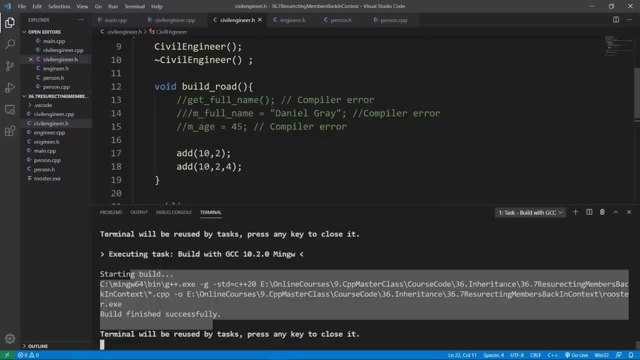 so the web is good and we are all fine here. this is really all i had to share in this lecture. i hope you found it interesting. we are going to stop here in this one. in the next one we're going to explore how constructors work with inheritance. go ahead and finish up here and meet. 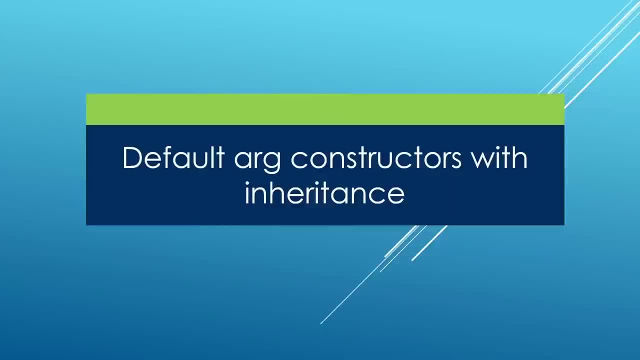 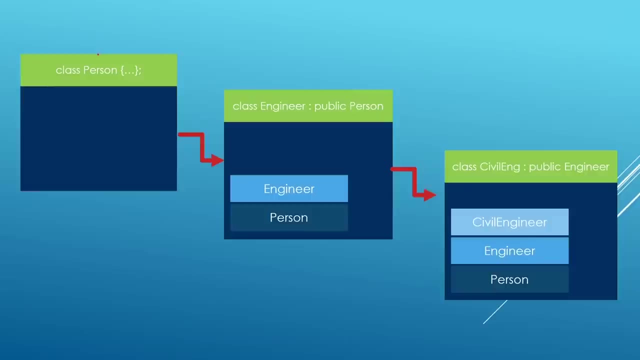 me there. in this lecture, we're going to zoom in at how derived objects are bought and we're going to zoom in on the constructors that we have been ignoring on purpose so far. so here we have the inheritance hierarchy we will be using. it is what we are familiar with at this point. 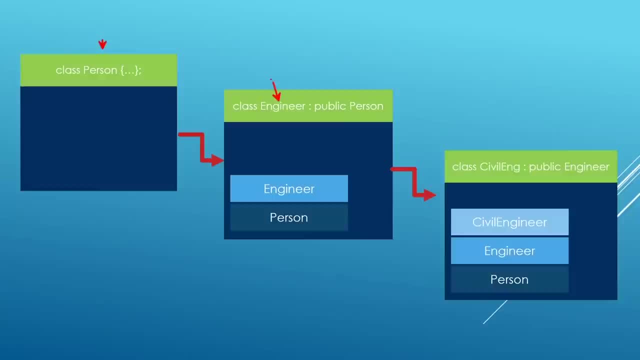 we have a person class which is going to be our base class. we have an engineer class which is now going to be doing public inheritance, because we have seen enough of private inheritance. our engineer class is now going to be nice and say: i am inheriting from person, but i also want my 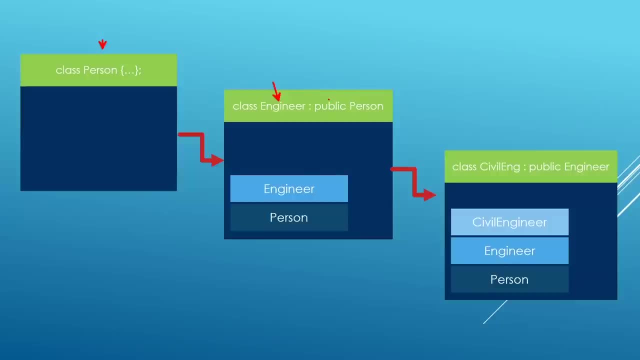 downstream classes to have access to the cool stuff i am getting from person. this is how our engineer class is behaving now. we are also going to have a civil engineer class, which is going to publicly inherit from engineer, but what we want to focus on here is what we get from bases. 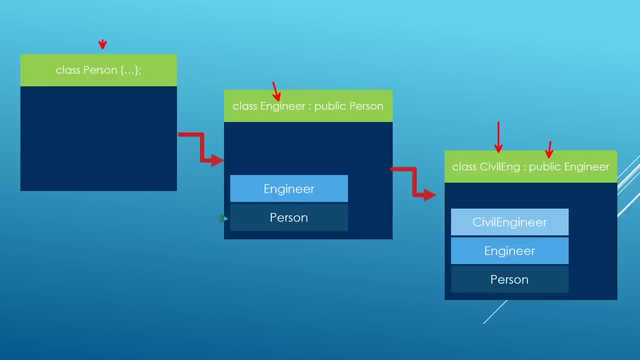 classes. so the engineer class is going to have a person part of that. but what we're going to have is what we get from base classes. so the engineer class is going to have a person part of that. but if you don't even have an ingénieur class, then you don't have training for the number. so, okay, okay, Πίθιμο. 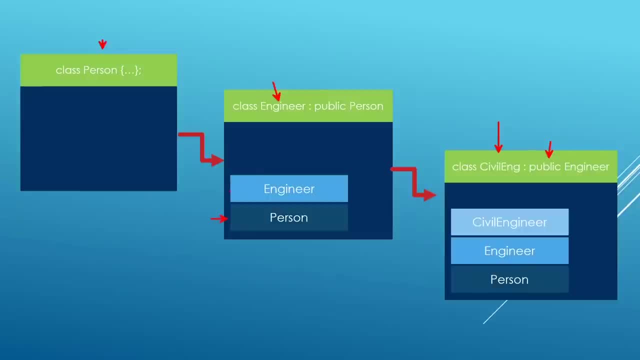 it is also going to build on top of that and add an engineer level and customize what kind of person it is. so if we inherit from engineer and weld our civil engineer class, the first thing to be built by c plus plus is the person part of this. it is going to weld an engineer level of this and then 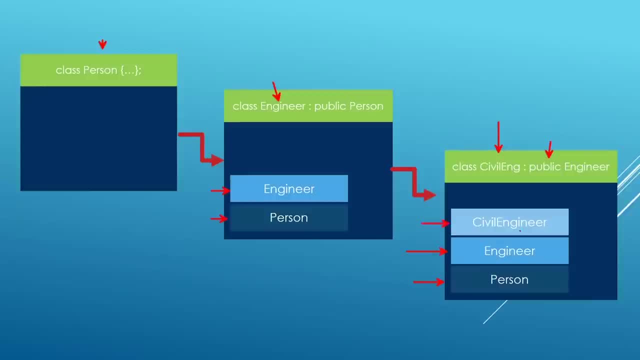 we are going to add the civil engineer level, to add the customizations that the civil engineer class is adding, and a, c plus plus is going to do this using constructors by default. we are going to be using default constructors if we don't specify a way for the base constructor to be called. 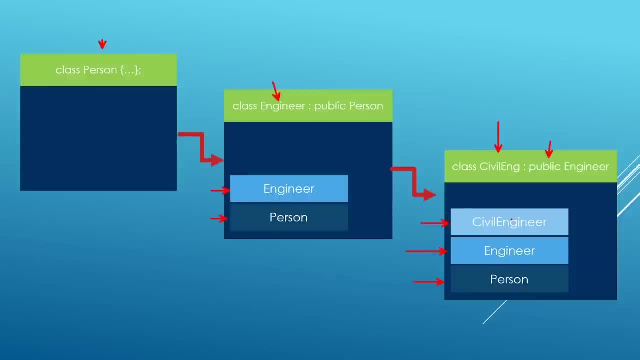 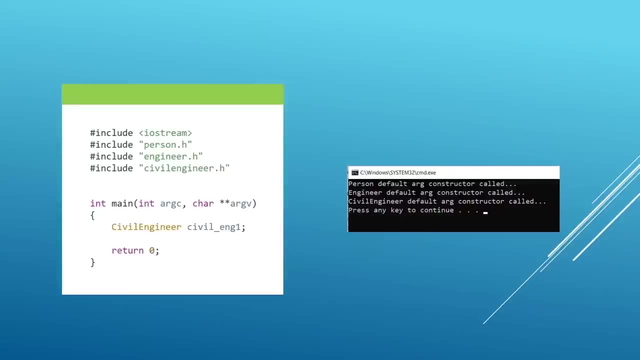 c plus plus is going to call the default constructor to build your base objects. so if we set up something like this and try to run our program, we're going to get output like this: we're going to see that the person default constructor is going to be called first and then the person 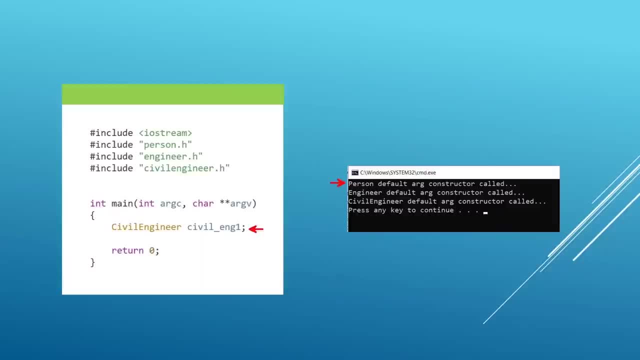 constructor is going to be called. second, notice that we are building a civil engineer object, so the default constructor for the most base class is going to be called. then we're going to be building an engineer layer on top of the person stuff that we get. then we're going to build a. 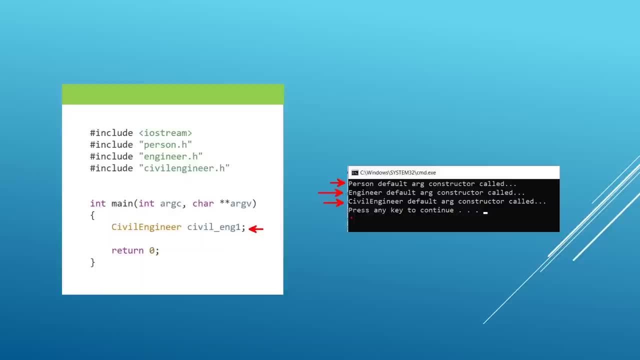 civil engineer layer on top of the engineer stuff that we have already got, and the compiler is going to do this using the default constructors by default. so we're going to call the default constructor first, we're going to call the default constructor for engineer, and then we're going to 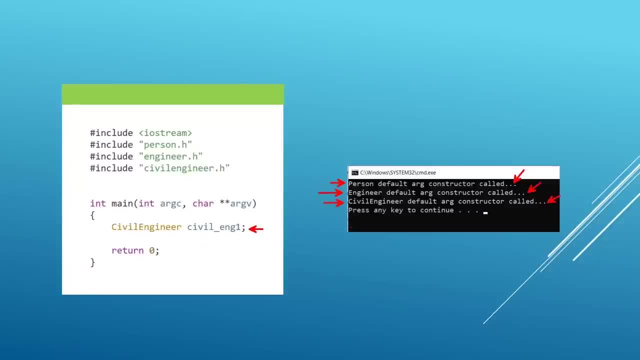 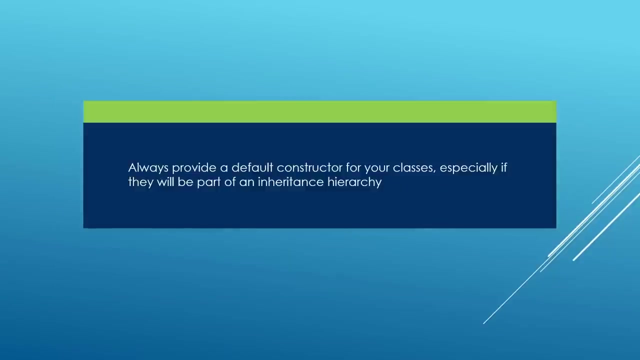 call the default constructor for civil engineer to complete the construction of our object. the object will be complete at this point and we will be able to use it later on in our program here and hopefully this is going to drive the point home that you should really really always provide. 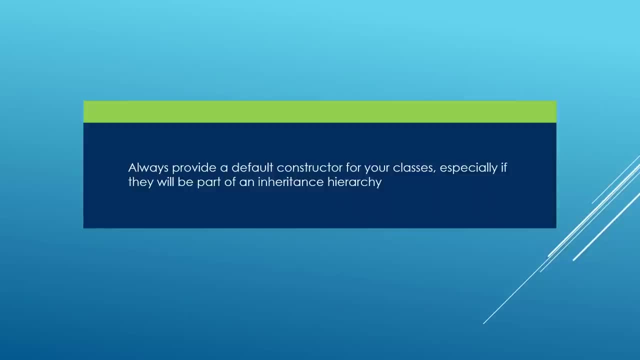 the default constructors for your classes, because the compiler may call this default constructors in unexpected ways, especially if your class is part of an inheritance hierarchy. for example, if somebody tries to build the civil engineer object and you don't have a default constructor for a person, the compiler is going to try and code that and it's not going to find that. 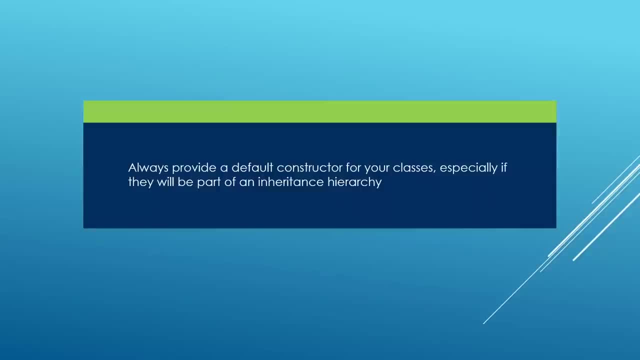 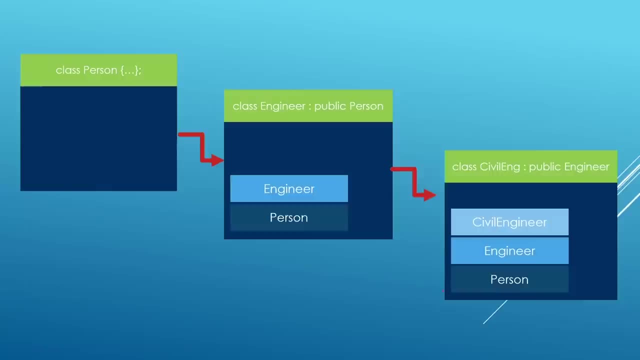 and it is going to throw a compiler error, as we are about to see in a minute. okay, so the message really in this lecture is that the most basic part of your class is going to be built. so, for example, for our civil engineer class, we're going to build the person port first, then we're going to 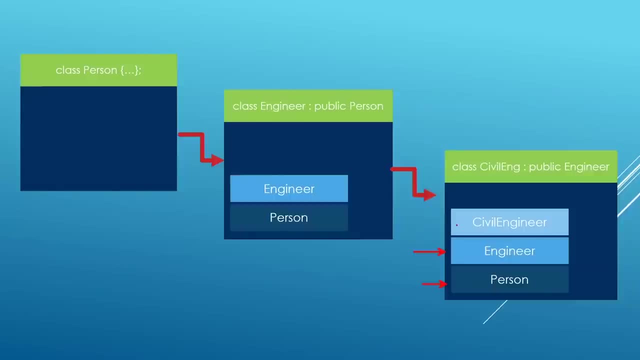 build the engineer part, and then we're going to build the civil engineer part of that, and then we're going to finish the construction of our object. this is the message here. now that you know this, we're going to head over to visual studio code and play with this a little more. 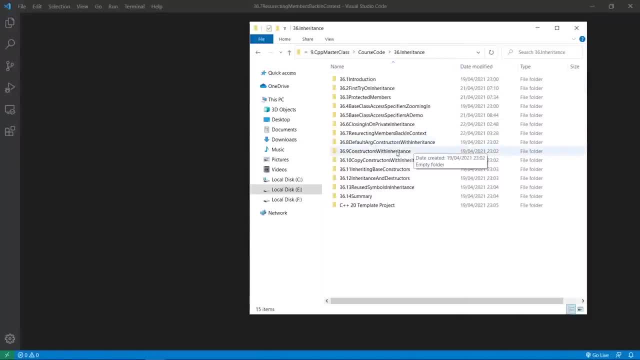 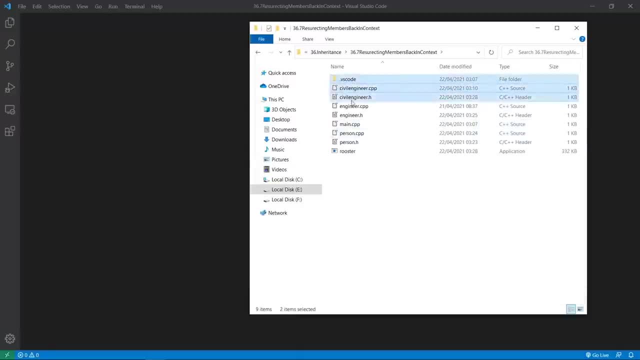 here we are in our working folder. the current project is default argument constructor with inheritance. we are going to reuse the argument constructor and we are going to use the argument code from the last lecture, because that's going to give us the classes that we need to play. 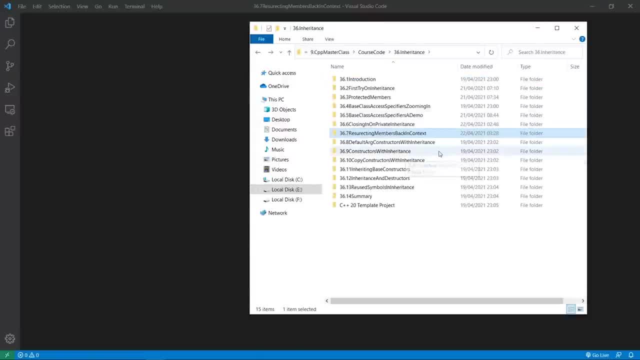 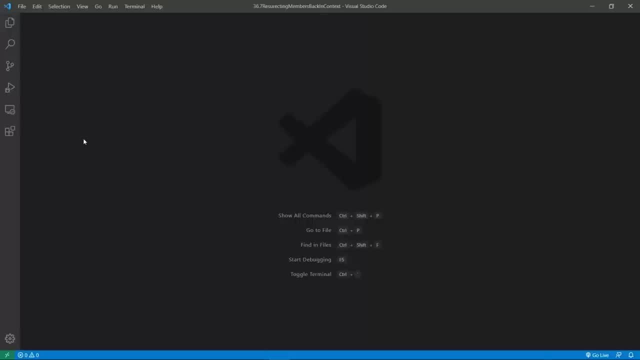 with what we want to do in this lecture, and that's playing with default constructors. let's put in our starter code and we're going to open this little guy in visual studio code. let's do this. so we're going to have our classes, we're going to have the main function which we can play with and we are. 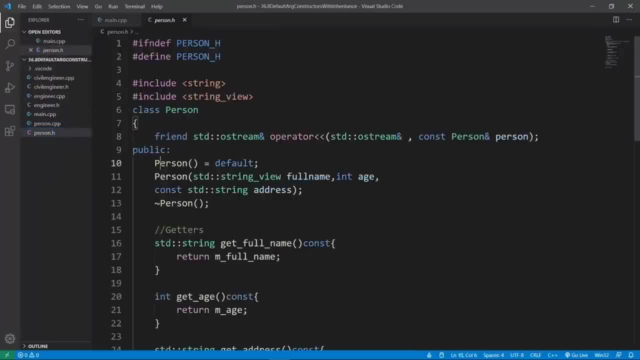 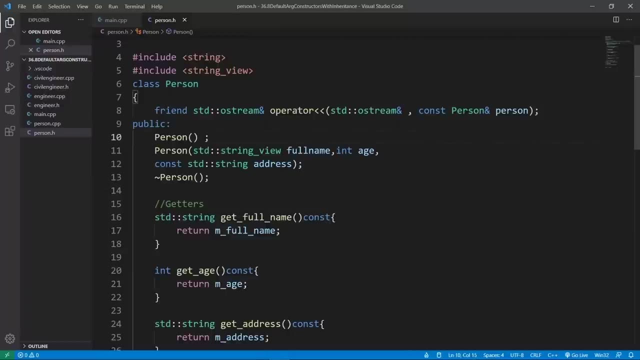 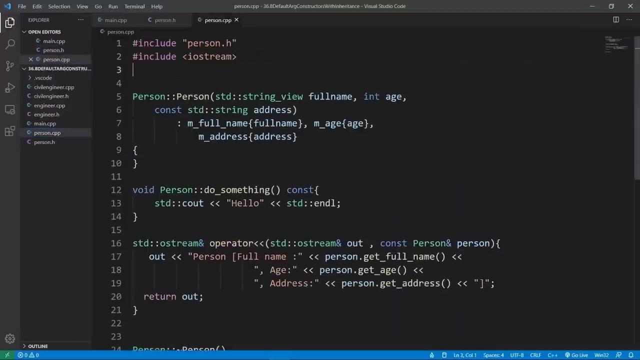 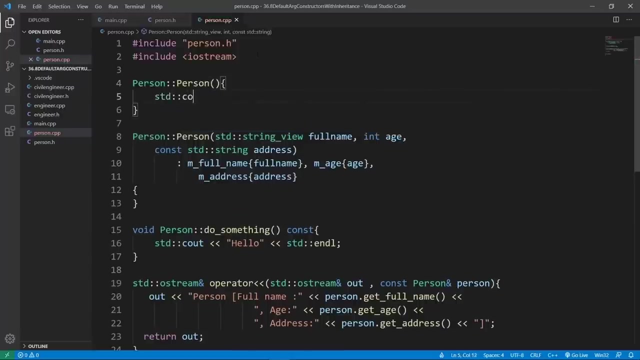 going to look at the person class and make sure we have a default constructor. we are not going to go to a file script. in the scripts that we built, let's say what makes incoming a counter. okay, so I'm going to go to the vmface and then I'm going to load the CSS very quickly. 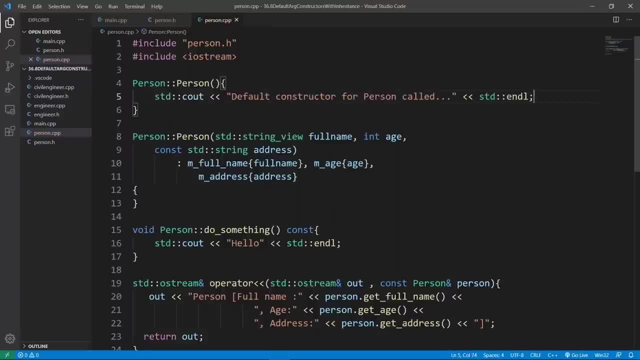 so what we're going to do is we're going to verify what we have been doing in this case, and what we stands for is our. a later policy should be a person like grandma's DS creation, which is a string of the JSON principles. this string types, this string types, this string typesota. 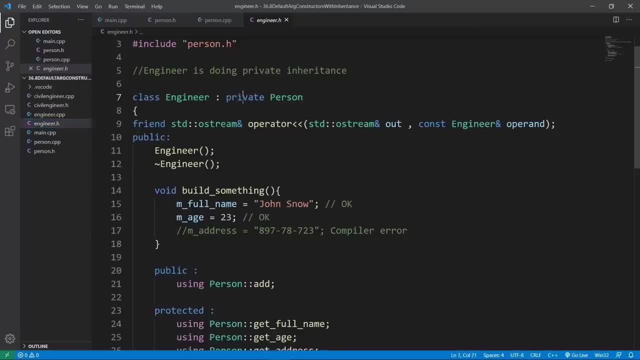 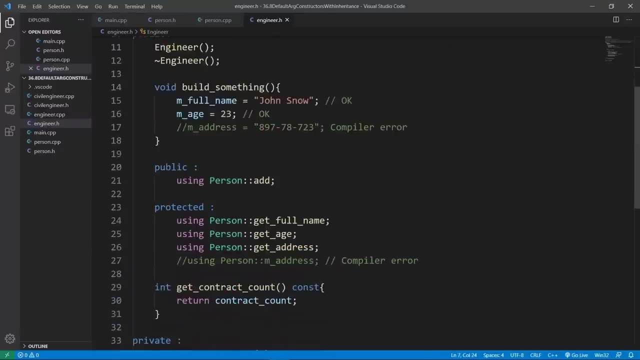 going to go to our engineer class and we're going to change it to do public inheritance. i think this is going to be much easier to deal with now and we're going to remove all these resurrection we were doing here from the last lecture, because this is no longer going to be. 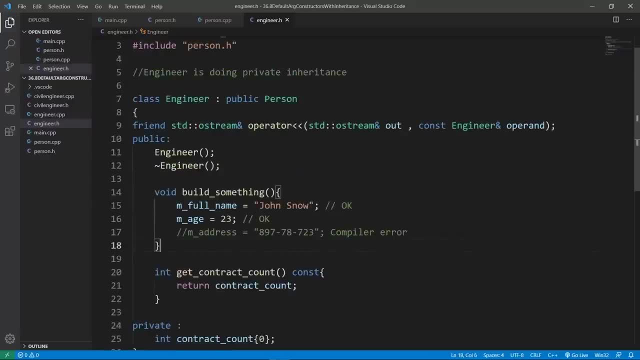 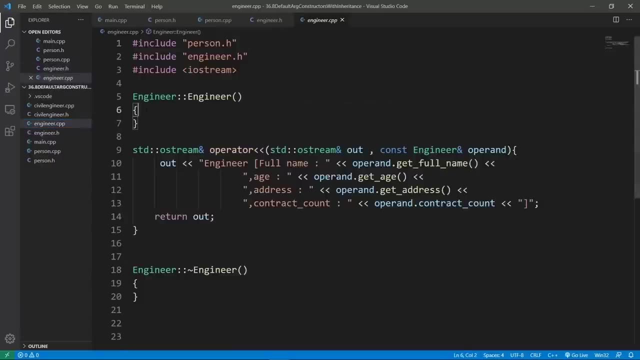 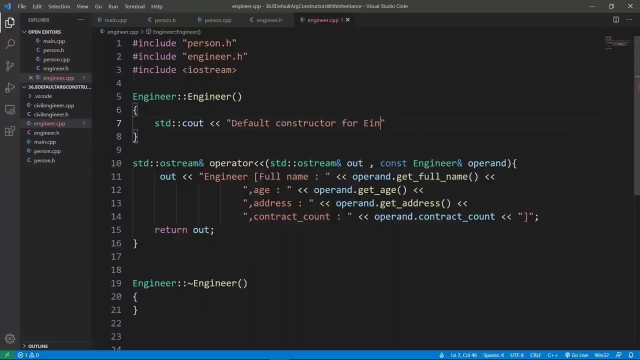 needed and what we really want is to look at our default constructor, which is really in here already. let's look at the implementation. all we really need to do is put in stdc out and say default constructor for engineer called and we're going to hop over to the civil engineer. 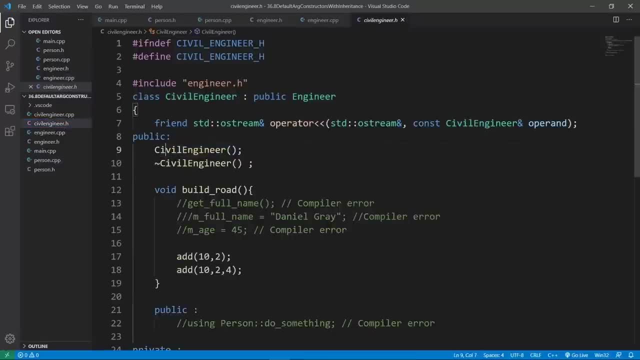 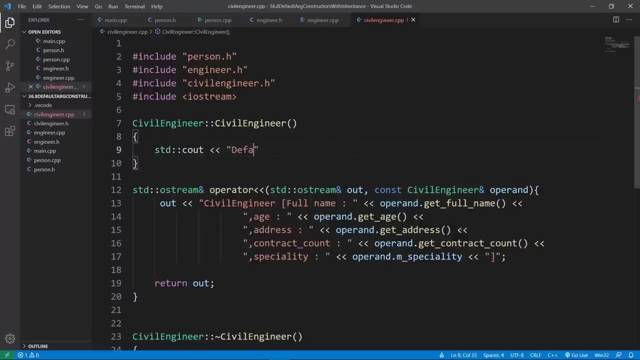 class and see if we have a default constructor. and we do have it and we're going to go to the cpp file and say: stdc out default constructor called for civil engineer. so this is going to basically do what we want and what we really want to see. 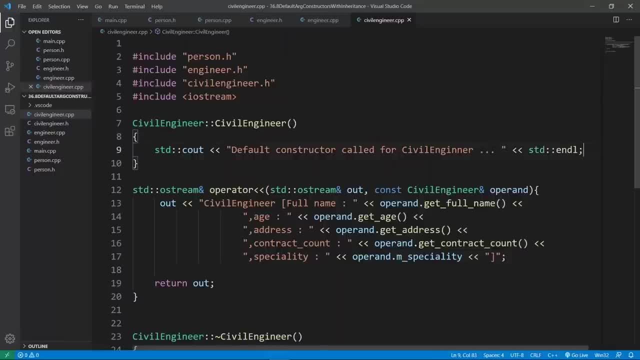 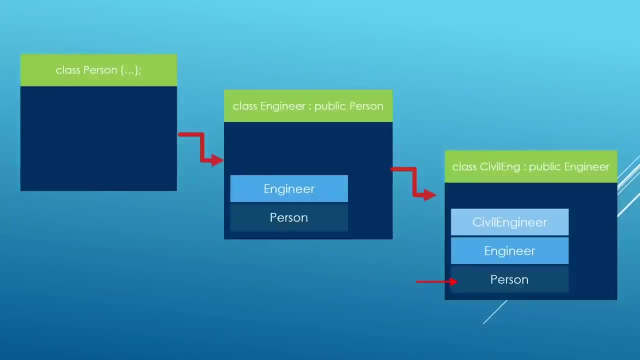 is how or the order in which our constructors are going to be called. if we build a civil engineer object, as we have seen here, the person part is going to be built first. so this is going to call the constructor from person and because we are not doing any kind of customization on which. 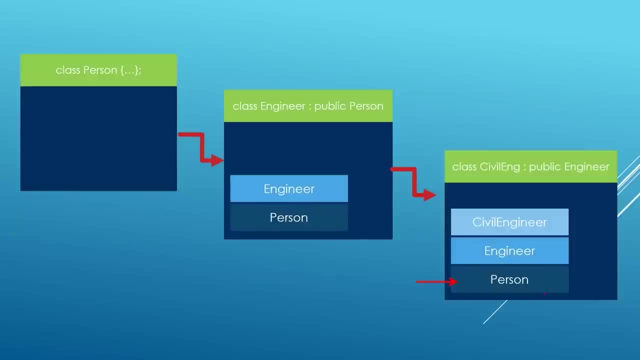 constructor is going to be called. the compiler is going to call the default constructor by default. so we're going to build the person port first and we're going to see the default constructor for a person called after that. we're going to build the engineer part of us and this is going to call the default. 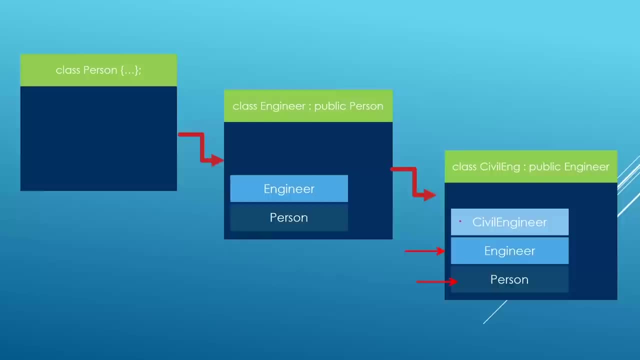 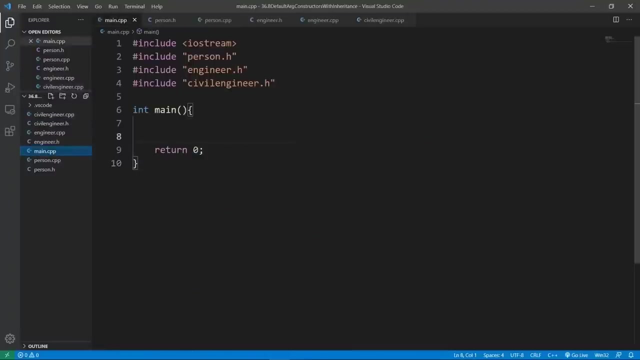 constructor for engineer and after that we're going to weld the civil engineer part of us and that's going to call the civil engineer default constructor. this is what we want to see if we build a civil engineer object. so we are going to hop over in the main cpp file and actually build a. 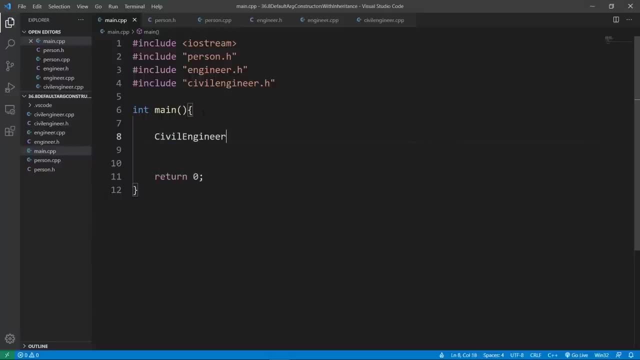 civil engineer object: we're going to say civil engineer and we're going to say ce1. we can do that and we're going to see what happens. let's try and build this program. we're going to build that with gcc. the build is going to be good, we can run it. let's bring up a powershell window. we can play. 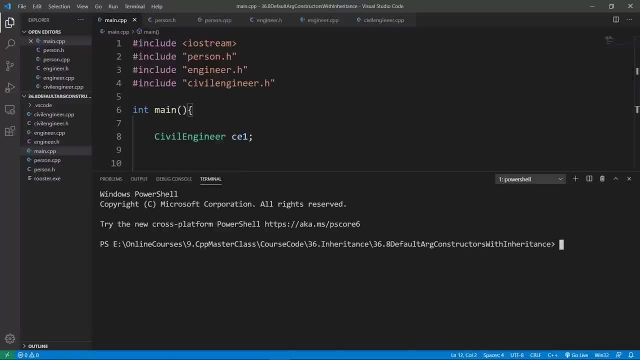 with. we want to bring up a powershell window. we can clear and run rooster and you're going to see the default constructor for person called the first constructor for engineer, called default constructor for engineer, called. this is what we want to see and hopefully this proves that. 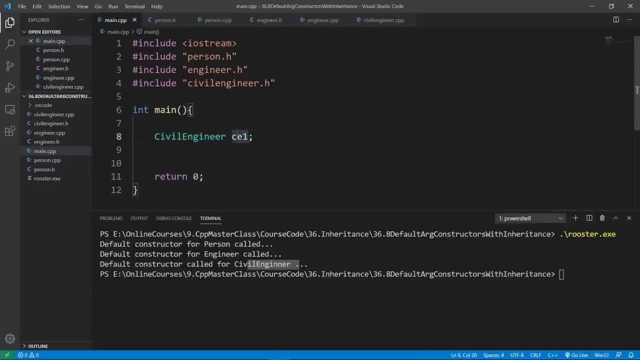 the compiler is really going to build our civil engineer object in parts. the compiler is going to see that it is a derived object and it's going to see all the classes that this is deriving from. so it is going to build the most base part first. after that it is going to build other layers. 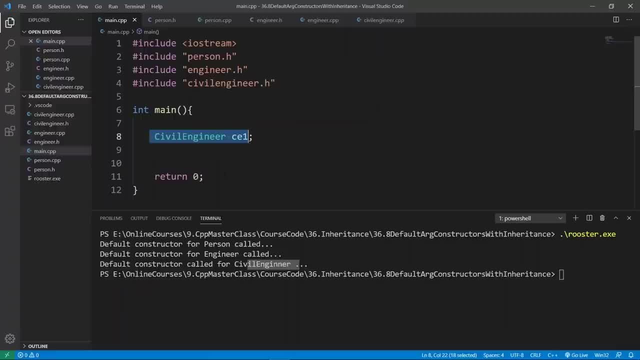 until it reaches the level where we are at at this. civil engineer objects. again, if we put another statement out here, we're going to say hello in here and we're going to say std, endl. and i am doing this so that i just have a point where i can put my breakpoint. some ides are not going. 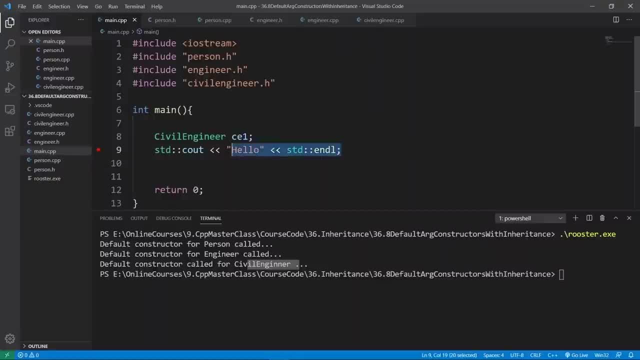 to like it if you put a breakpoint at an empty line. so that's why i am doing it here and i am going to try and debug and really show you that we have an engineer and a person part in us. i have shown you this before but it doesn't really. 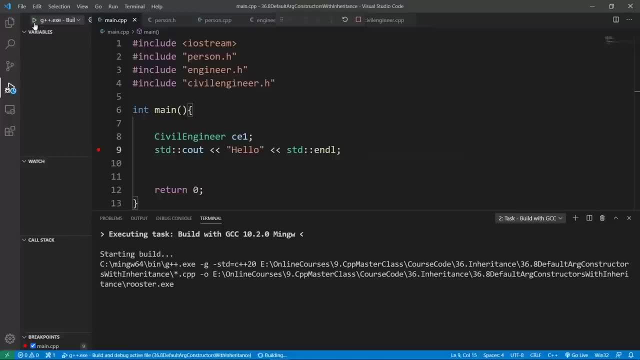 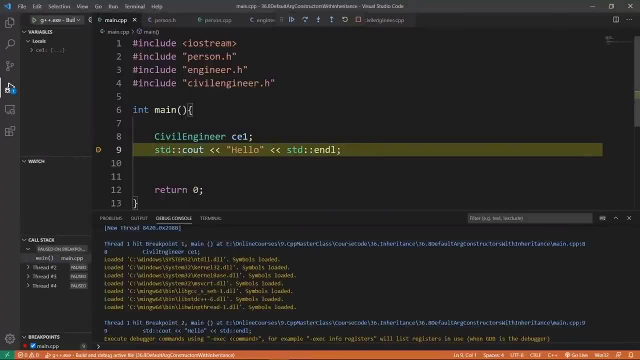 hurt to repeat this, because debugging is really cool. it's going to give you more information than you could ever ask for. we're going to hit our breakpoint here and, if we look in our locals, we're going to have our civil engineer object, which is in scope now. 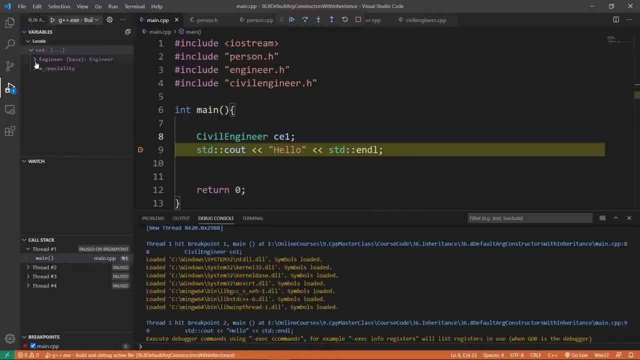 and you see that we have an engineer part of us and the engineer has a person part in it. so what the compiler is really going to do when it is welding a civil engineer object, it is going to weld the most base part of us, so it is going to build the person part after that. 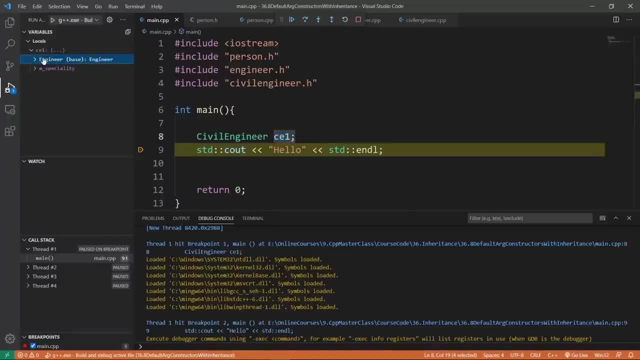 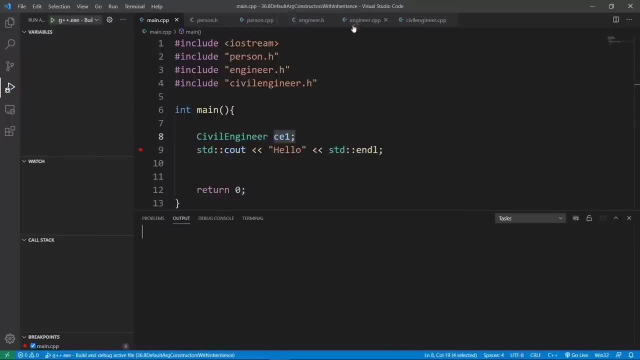 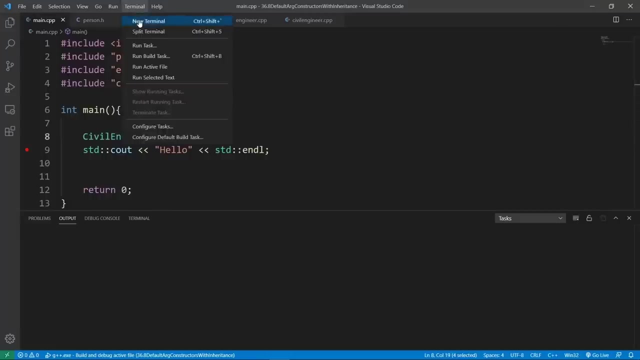 it is going to build an engineer layer on top of that and then it is going to weld the civil engineer layer and that's what we see in our output when we get to run our program here. if we go back, we're going to see that we still have our binary. we can still run it. let's bring up a terminal. 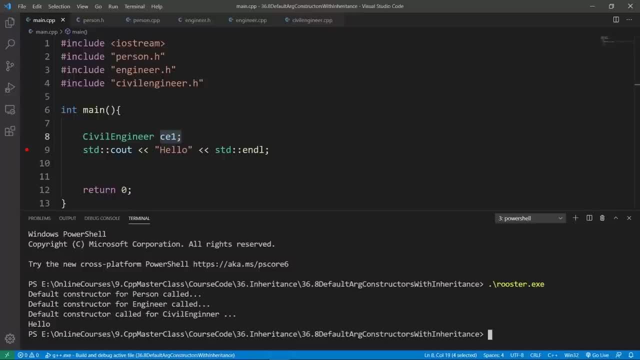 we can use to run this, we're going to run rooster and we're going to see the order in which our constructors are called, and this is really cool. now that we have just debugged this program, we can take out this hello line, because it's really useless and this is really what i wanted you to. 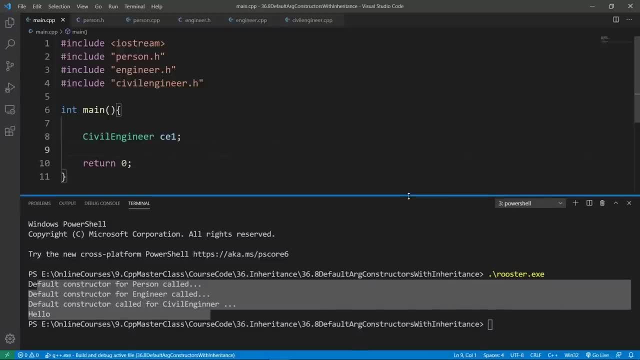 see, constructors are going to be called in your inheritance hierarchy, starting from the most basic, going down to the most specialized one. so we're going to call the most best constructor, which is person, and then we're going to call the most basic constructor, which is person, and then we're 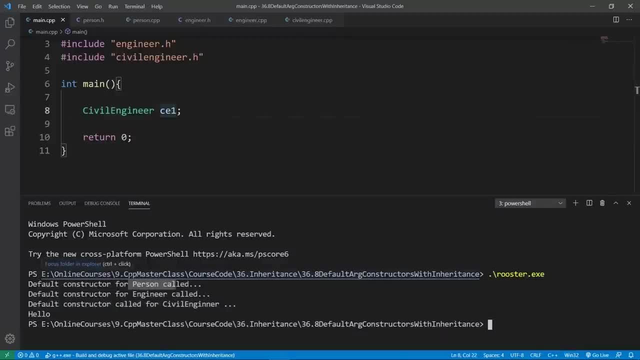 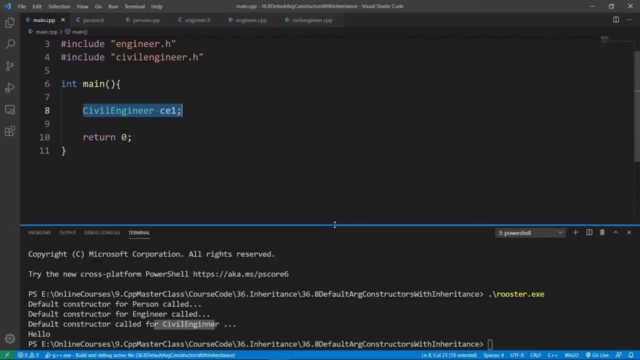 going to keep going until we reach the most specialized, which is a civil engineer here to build our object, and our object is really going to be boiled up in layers. this is the message i am trying to convey here. this is really all i had to share in this lecture. i hope you found it. 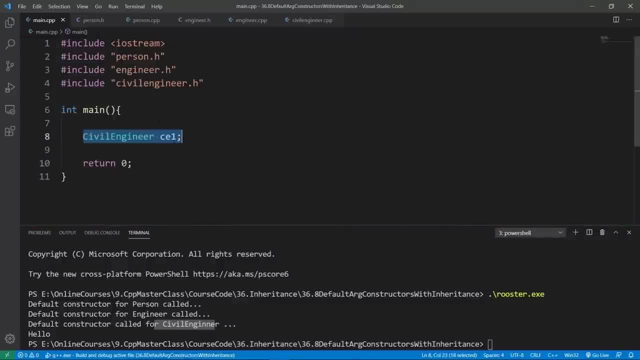 interesting. we are going to stop here in this one. in the next one we're going to see that we can actually actively call a base class constructor from our derived class, and that's going to add much more flexibility in how our objects are built. we are not going to call the 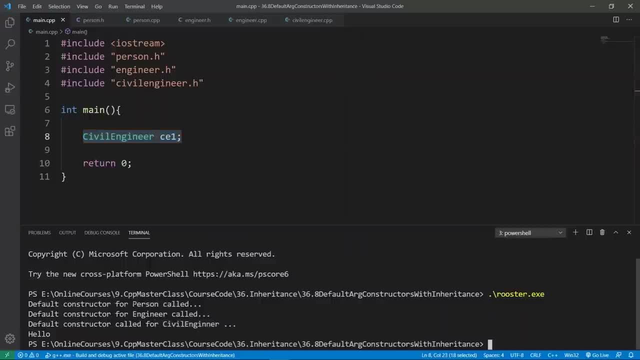 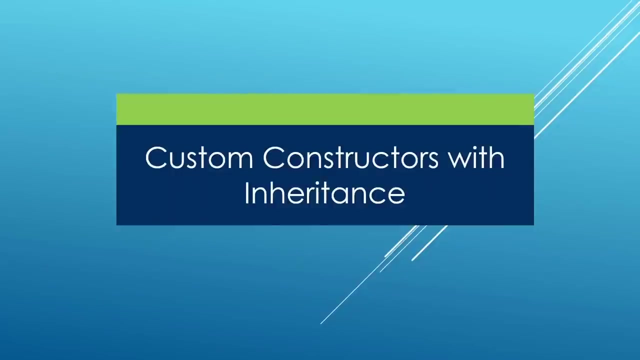 default constructor. we're going to be calling our own constructors and have much more control on how our derived objects are set up and built. go ahead and finish up here and meet me in the next lecture. in this lecture we're going to see a way we can instruct for custom constructors to be called. 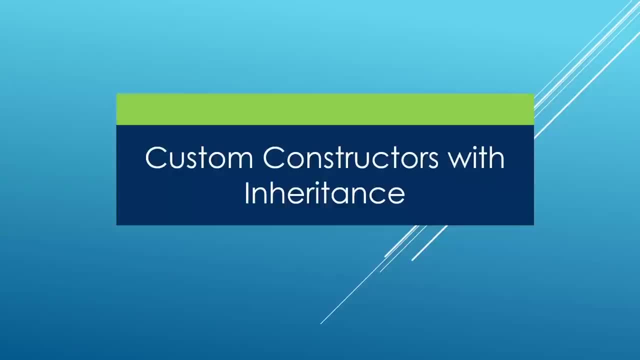 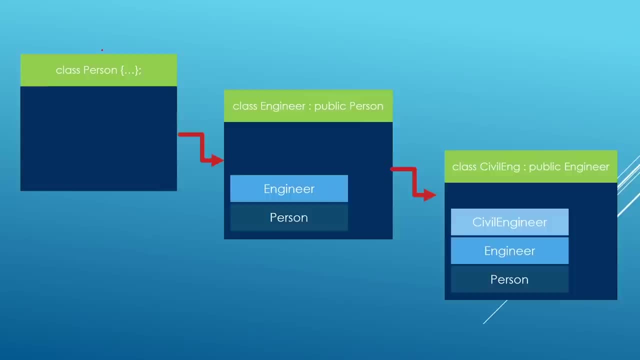 when our derived objects are being built, built and set up. in the last lecture we saw a figure like this. we had an inheritance hierarchy that went from person to engineer and to civil engineer and we saw that if we set up a civil engineer object, a person part is going to be built first, an engineer part is going to be built on top. 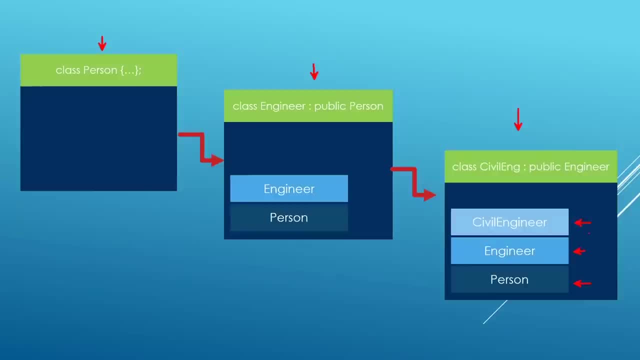 of that and the civil engineer part of that is going to be built and then we're going to have the construction complete for our civil engineer object. but in the last lecture we saw that this was calling the default constructors and sometimes you don't want this, you want your objects built in. 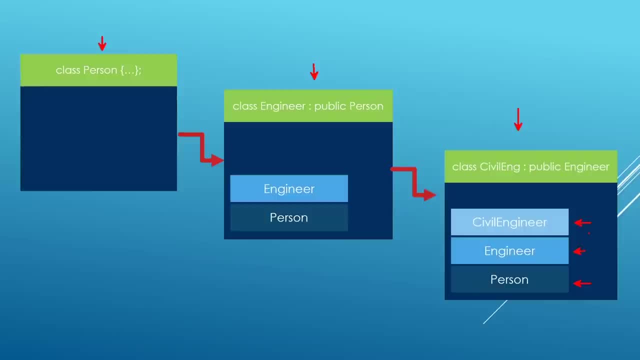 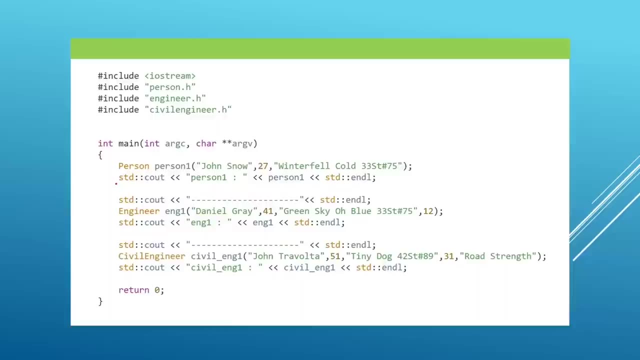 a specific way, for example, through a bunch of parameters that you passed your constructor. what, if you want this kind of setup? this is what we are going to learn about in this lecture, and what we want to end up with is something like this: we will be able to build a person object. 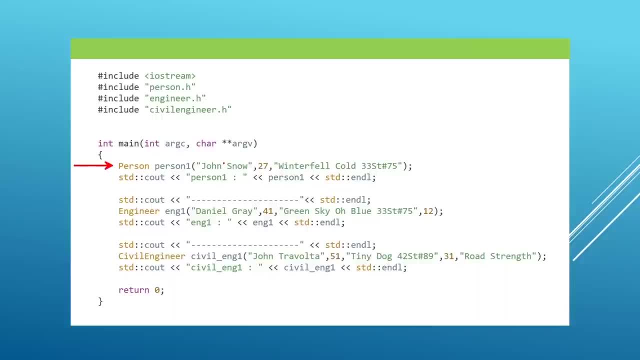 by passing in a bunch of parameters. we can pass in the full name, we can pass in the age- i think this is the age we can pass in an address. we can build an engineer object by passing in this kind of information. we can pass in the name, the age and the address, but we can also pass in 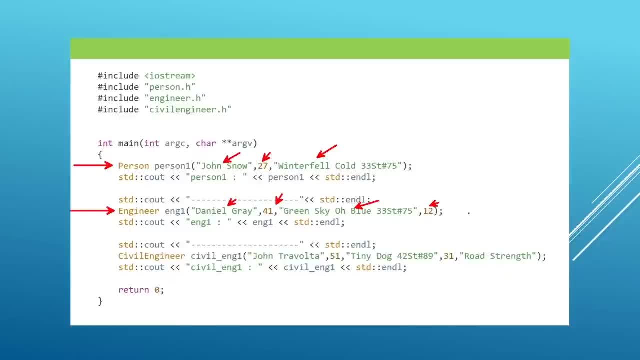 the contract account. i think this is the new member variable we had in our engineer class. but we're not going to stop there. we can also build the civil engineer object and we can pass in the information again, as evil engineer is also a person. so we're going to be. 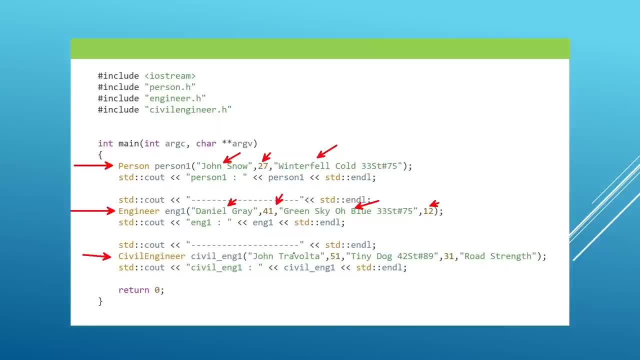 passing the information that is going to initialize the person part and that happens to be the name, the age and the address. but a civil engineer is also an engineer, so we're going to pass information that portrays through the level of an engineer and that's going to be the contract count and we're 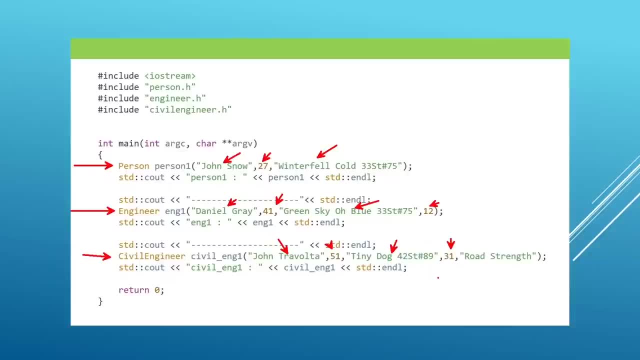 going to pass the information to initialize the civil engineer part of this object and that's going to be the road strength and hopefully from this you can see that we need a way to forward all this information to the constructor where this information is needed, for example, if we are balding a. 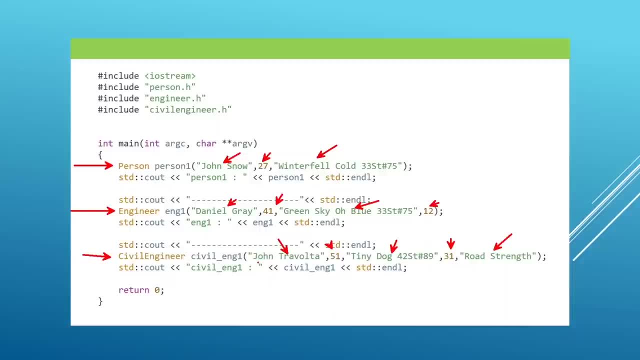 civil engineer. object: we want to forward the name, the age and the address to the person- part of us- so we need to process to our personal constructor. in a way, we need to pass the 31 here to our engineer constructor, because this information is going to be stored at our engineer level and we need to store the road. 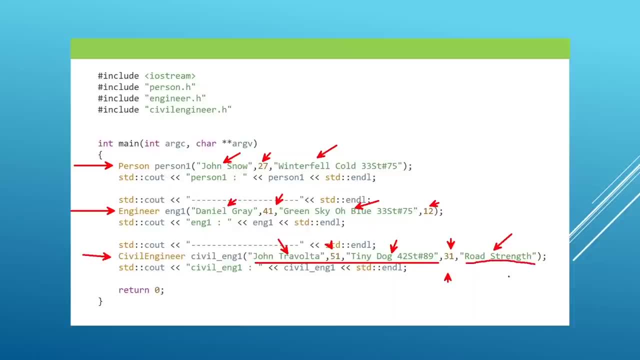 threats information into the civil engineer part of us, because that's where this member variable is declared. hopefully you can see the need to call custom constructors, which are not to default. these custom constructors are going to allow us to forward information when building our objects, like we are. 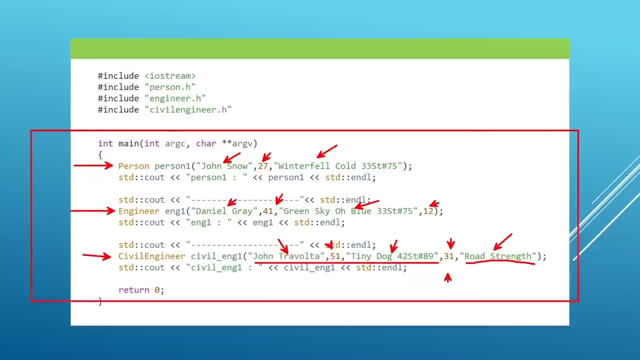 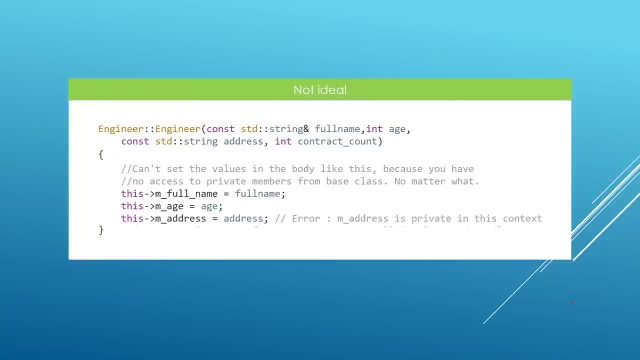 doing here in the main function. so let's see how we can do this. some of you might think, uh-huh, if I am building an engineer object, I can just grab the information and pass that to my base class, and that is simple, right? so we can. 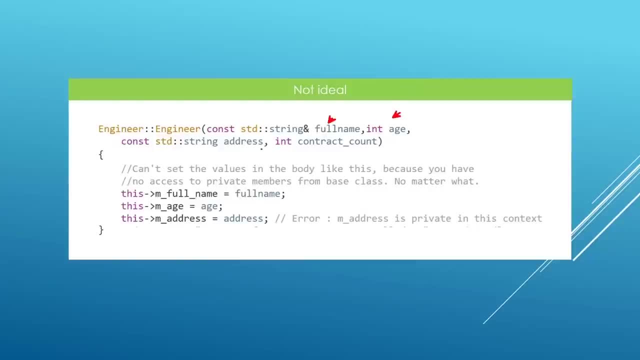 grab all this information. we can grab the full name, the age and the address and pass that to our base class using the syntaxes we have here. if we are doing public inheritance, we're going to have access to these guys anyway. so we can say full name equals full name, M H equals age and say M address equals. 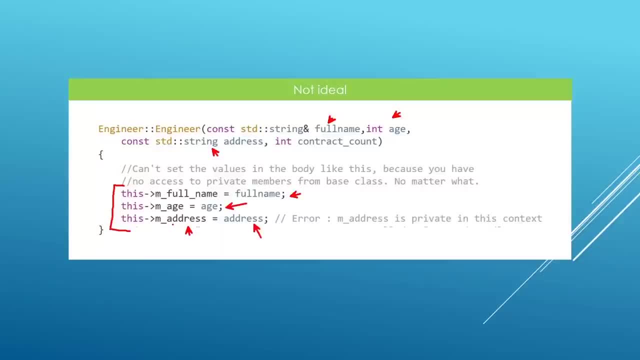 address you, except for the address is actually private to the person class, and we can't do something like this. if we try to access the address member variable from the base class and modify it, we're going to get a compiler error that says that the address is actually private to the base person class. we can't do this, so. 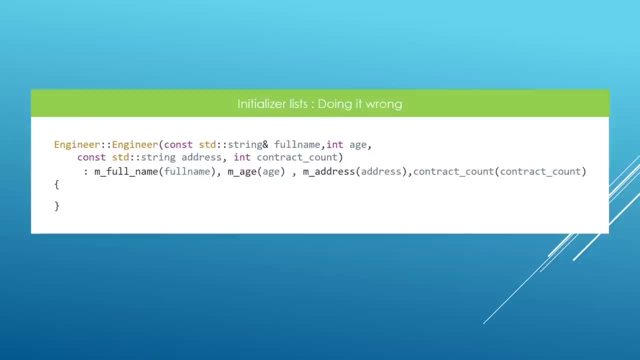 this is not going to work. okay, some of you might think, uh-huh, what if I try to use an initializer list and do something like this, so I can say M full name and pass in my information. I can say M age and put in my information. I can say M address and put in my. 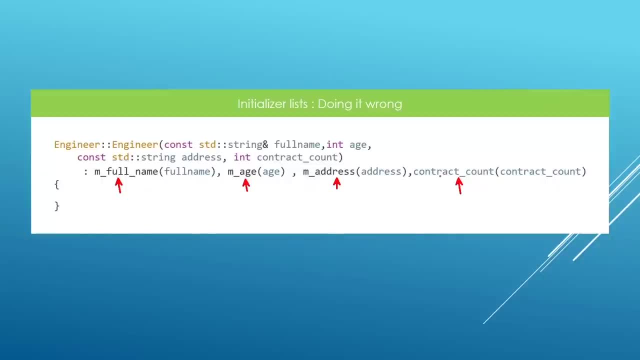 information and then initialize the member variable that actually belongs to the engineer class that we are trying to build an object for here, and hopefully this is going to work, except the compiler is not also going to accept this. the reason is, with initializer lists you can't initially. 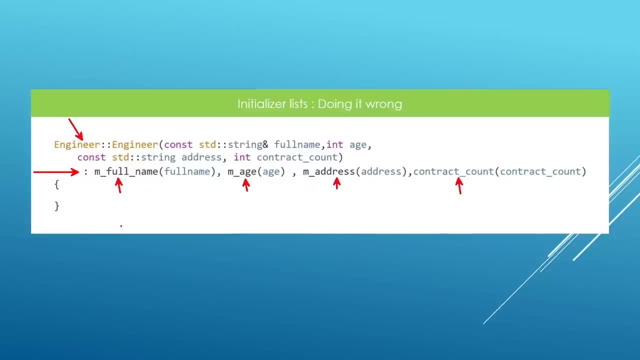 initialize a member variable that doesn't belong to the class that you are trying to build an object for. so, for example, here we are trying to initialize M full name, M age and M address, but this member variables don't belong to the engineer class that we are trying to build an object for. so we're going to 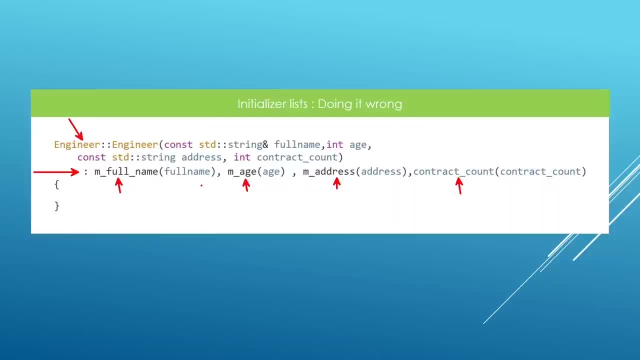 get a compiler error here. this is not going to work. it is not engineers job to build or set up this member variables, so this is not going to work, okay, so? So how are we supposed to forward information from derived classes to base classes? Not to worry here. 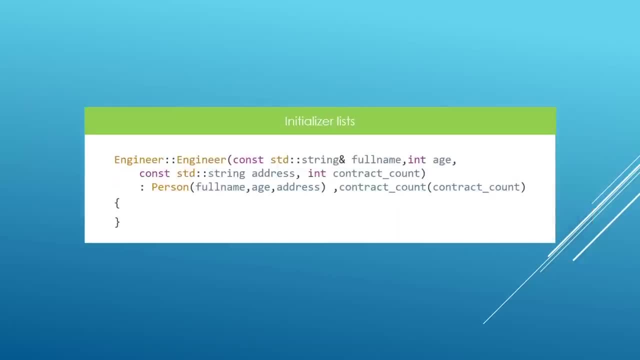 We can still use initializer lists, but we are going to use constructors whose job is going to be to initialize these member variables. So if we are building an engineer object and we have information that really belongs to the person part of us, we're going to call the person constructor to actually use this information. 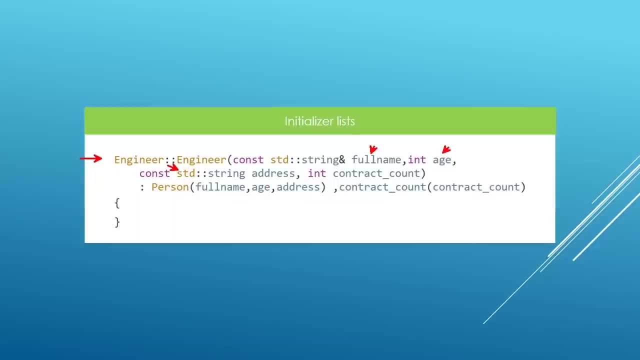 to build the person part of us And we're going to be calling the person constructor in our initializer list here And after we do that, we're going to initialize a member variable that actually belongs to us in our initializer list And this is going to forward information from derived classes. 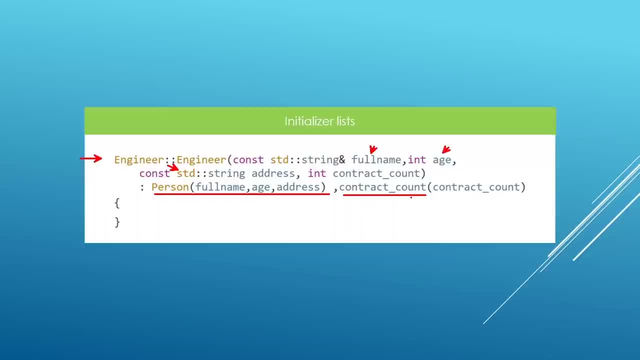 In this case, the engineer is the derived class and the information is going to be forwarded to the person constructor, which is our base class. This is how this is going to work. Okay, Now that you know this, we're going to head over to Visual Studio Code and play with this a little. 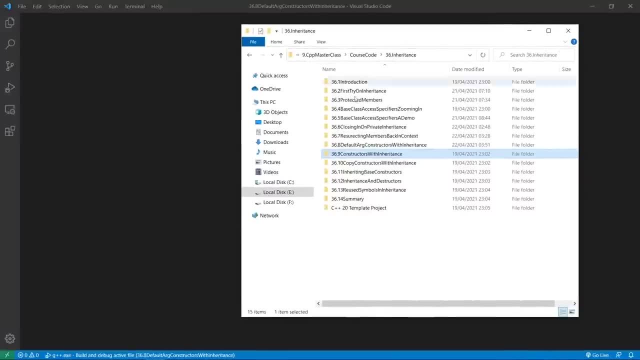 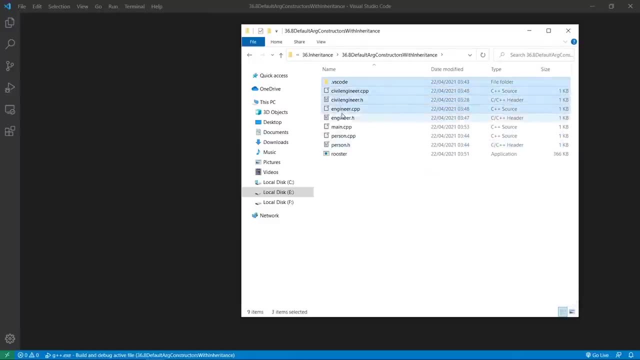 more. Here we are in our working folder. The current project is constructors with inheritance. We are going to grab the code from the last lecture because that's going to be our starting point, And we're going to paste this in our current project. 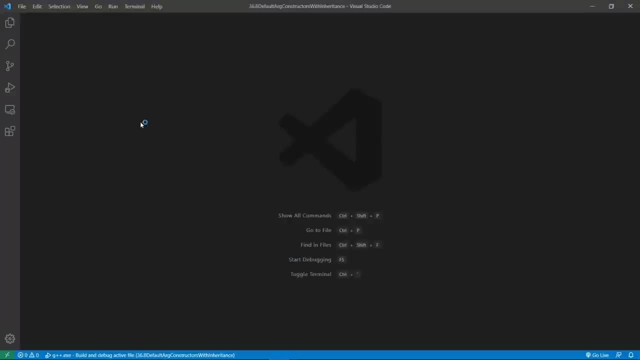 We are going to open this little guy in Visual Studio Code by dragging and dropping here, And this is going to give us our starter code. We're going to have a person class, an engineer class and the civil engineer class, And this is basically going to set up the hierarchy we have here. 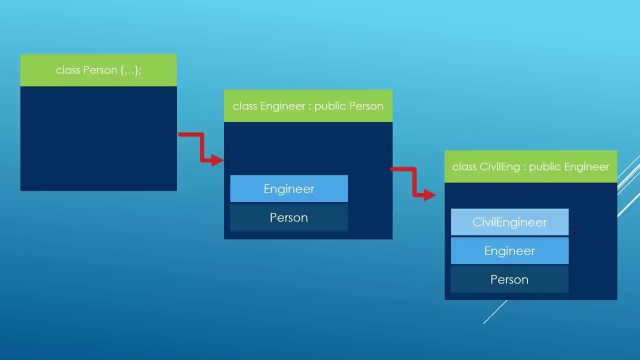 And what we want to achieve is to be able to call our own custom constructors When we build our object in layers. information is going to be coming from a civil engineer object And we are going to initialize the person part of us with relevant information. 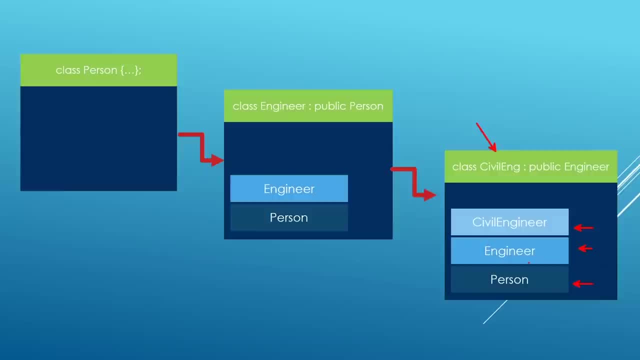 We're going to initialize the engineer part of us with the relevant information And we're going to initialize the civil engineer part of us with relevant information. This is what we wanted to achieve. Okay, For that to work, we need to not call default constructors. 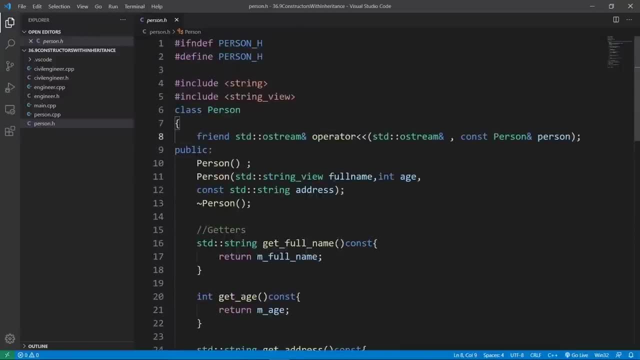 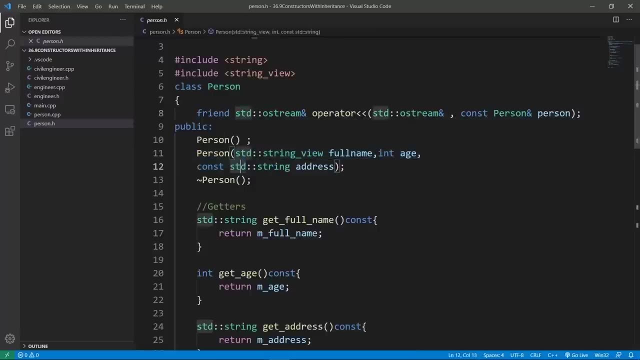 We want to call actual constructors that are going to grab the information and forward that in our member variables. For example, in person we have a constructor which is going to take three pieces of information and it is going to pass this information into our member variables. 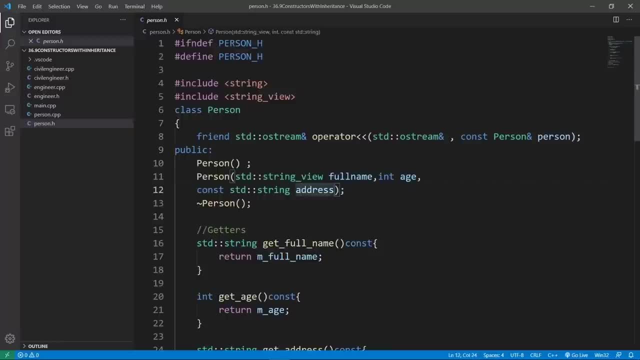 And this is what we want to build in our project. Okay, variables: we need to apply a few changes here. for example, our third parameter is passed as a cost string member type. we are going to change this to be std string view, because this is going to save. 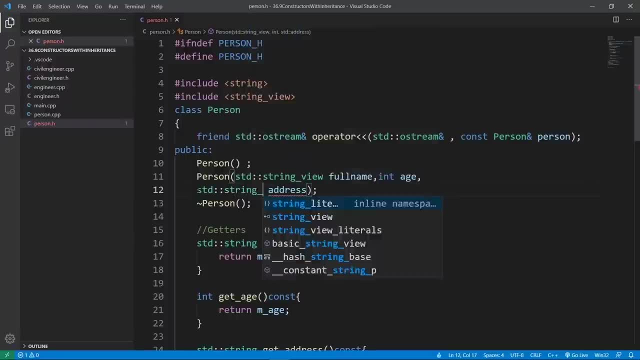 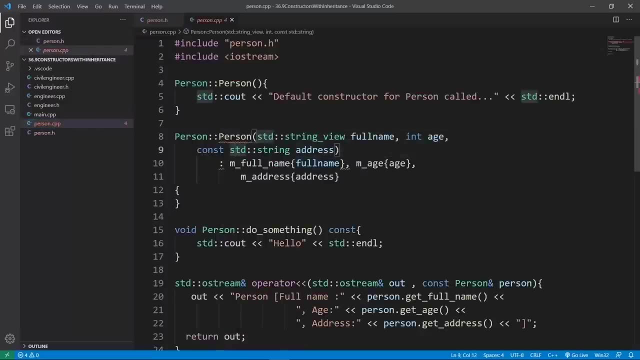 us on copies. let's say string view here. this is going to work and this is going to forward information in a way we want. we're going to change our third parameter to be std string view. let's say string view here. we're going to say std string view. this is what we have in our header. 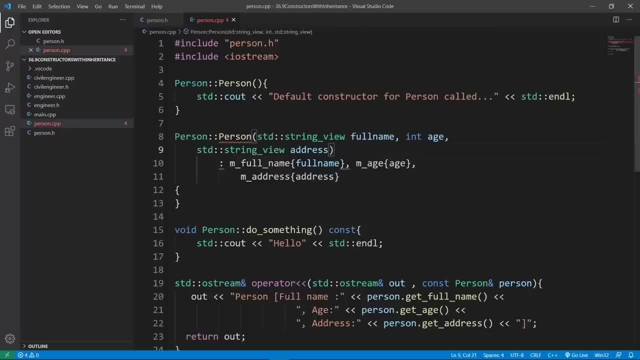 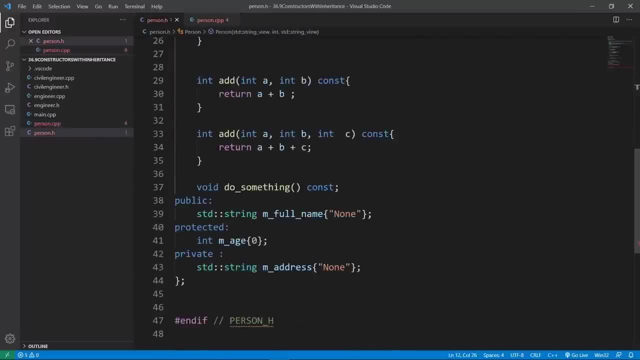 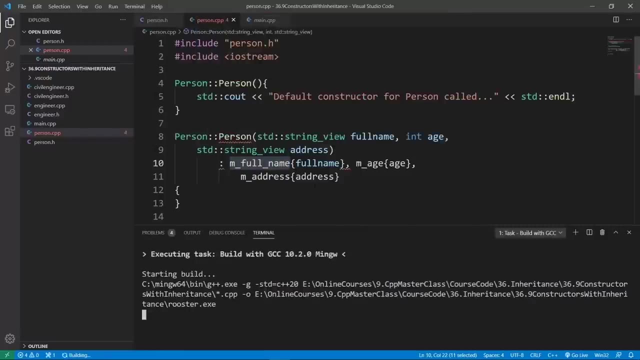 we're going to be having the same signature for our function here. and what is wrong? we have m full name, m h and we have m address here. let's try to build and see if the error goes away. sometimes visual studio code is playing games on us. if we get a compiler error, we're going to try and fix. 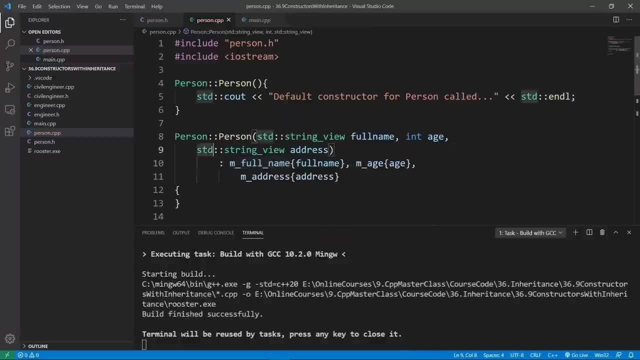 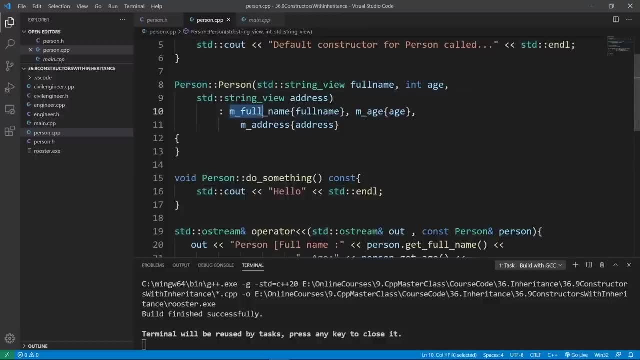 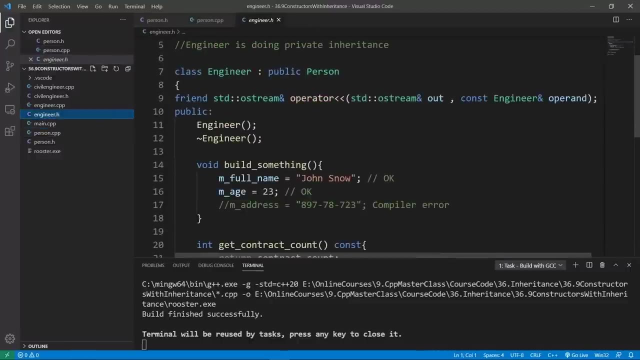 that you see that it is visual studio code playing with us. the code is just fine here. so we have our constructor for person. it is going to forward information using our initializer list. here we're going to look at our engineer class. if we go there, we're going to see that we don't have any constructor, which is 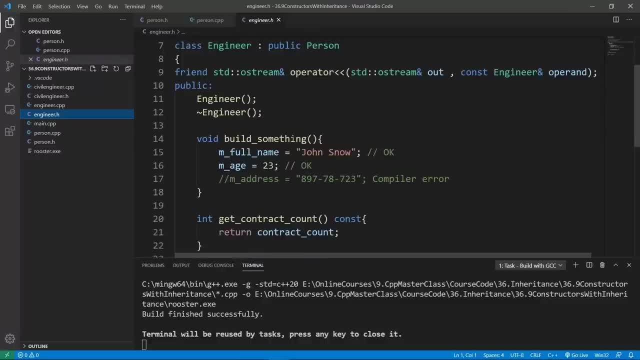 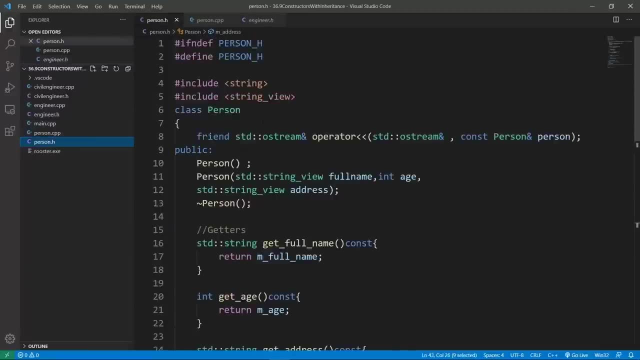 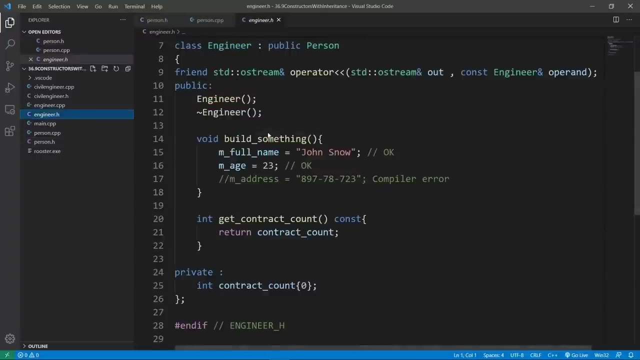 going to grab information in any meaningful way and put that in our class. so we are going to put in a constructor that looks like the one we have in our person class, so we can just grab this. i like copy and pasting, because that's going to save me a few seconds, so i am going to put my constructor here, only it is not going to be called. 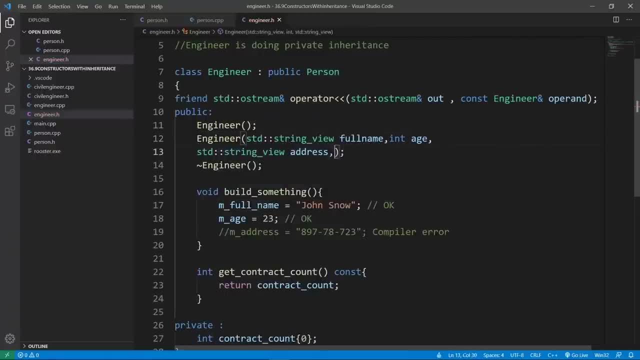 person. it is going to be engineer and i am going to add a construct count member and this is going to be an integer here to keep things simpler, and we are going to put an implementation of this constructor in our engineer class. we can go down here and we are going to put an implementation of 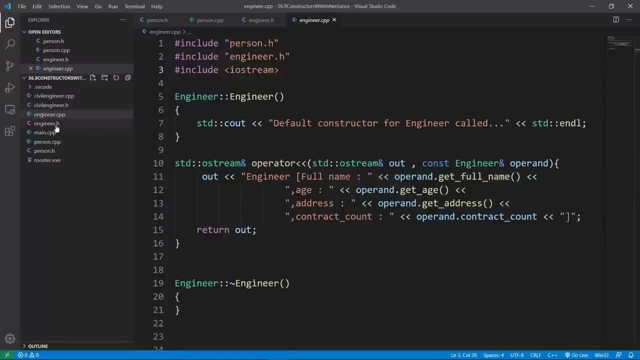 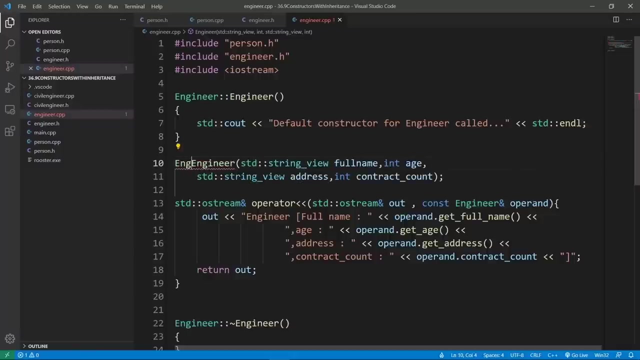 here and put that in front of other constructors. let's look at the order we have in our header, because i like to be consistent. the default constructor is first, so this constructor is going to be second and we're going to say that it belongs to the engineer class using a scope of 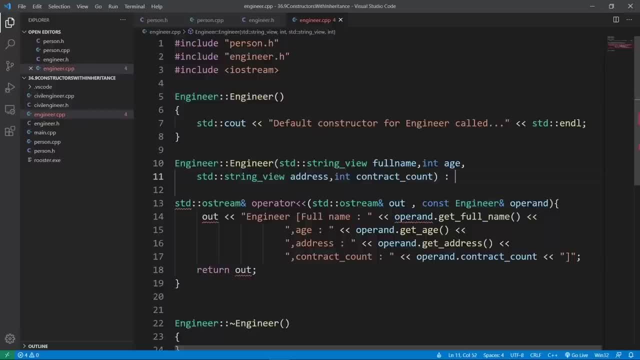 resolution operator here and we are going to put in our initializer list. now what we want to do is to call the constructor for person to initialize a person, part of us- and then we're going to grab the information for the contract count and we're going to forward that in our own member variable. the way we're going to achieve 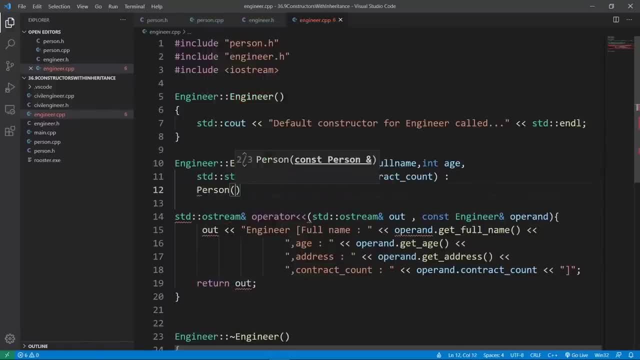 this: we're going to call the person constructor and we're going to pass in the full name, we're going to pass the age and we're going to pass the address, and then we're going to initialize our own member variable, which is contract count. i think let's go to the header and look at that. 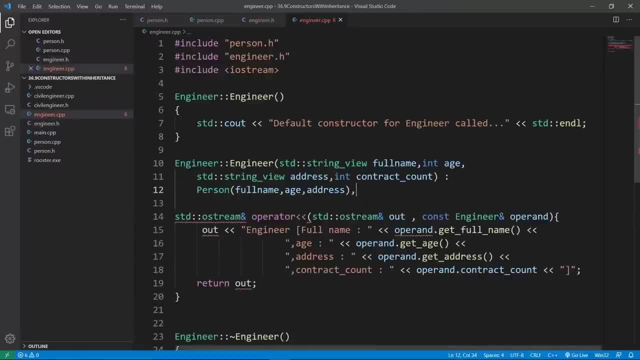 we're going to see that our member variable is contract count, so we're going to say contract count and we're going to say contract count param. we're going to name this differently because we don't want issues with naming here, so let's name our parameter here. 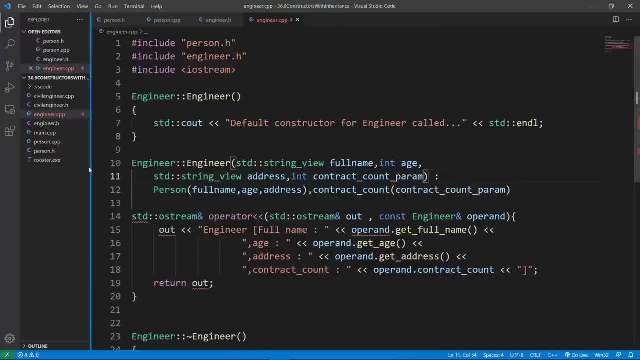 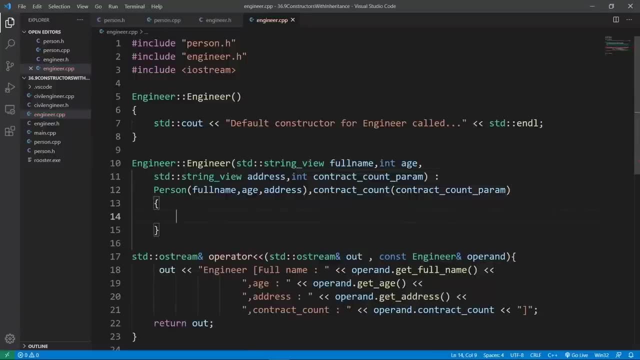 param. this is going to not confuse the compiler and once we have this end, we can just put in the body, which is going to be empty, because all the initialization is now done in our initializer list here. so if we do this, we're going to see that the compiler is going to be empty and we're going to 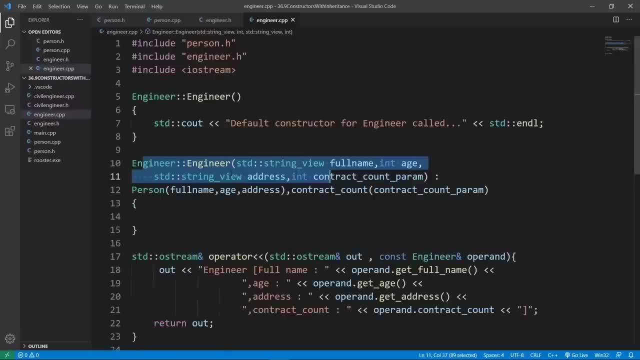 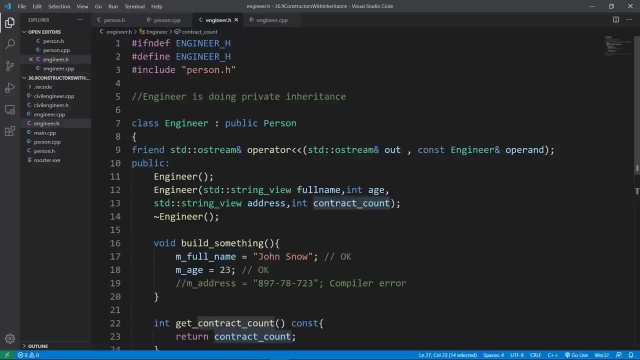 be happy with our thing here. we're going to go down in our civil engineer class and we're going to grab the constructor. we have an engineer because we're going to be using this as a starting point. we're going to copy it and go in our civil engineer class. we're going to see that. 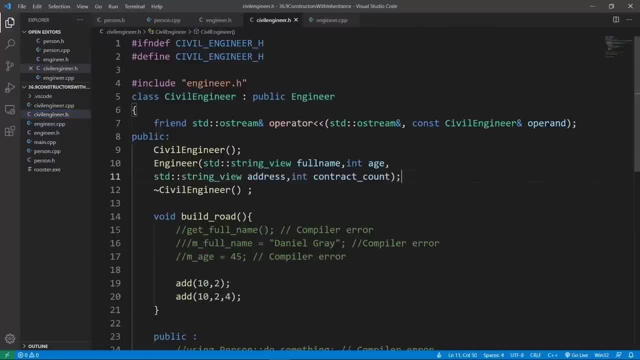 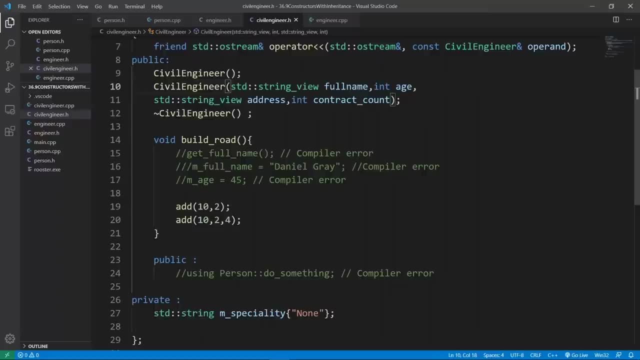 we don't have a custom constructor. we're going to put this in, we're going to name this civil engineer and we're going to add a speciality member that we want to initialize. so we're going to say std string view. because we want to forward string data, we're going to say std string view. 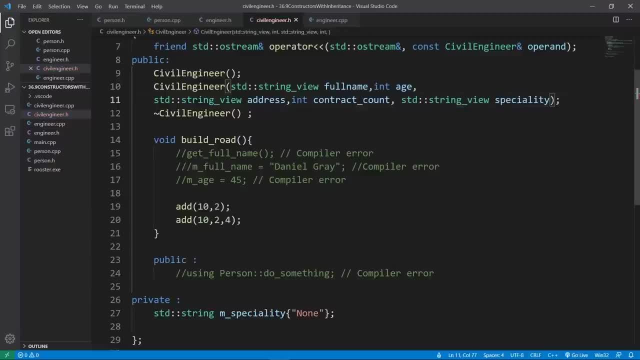 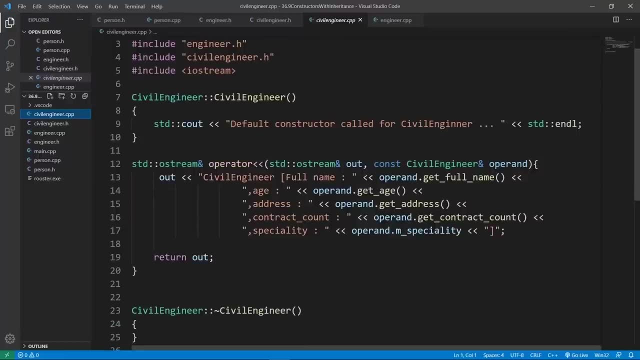 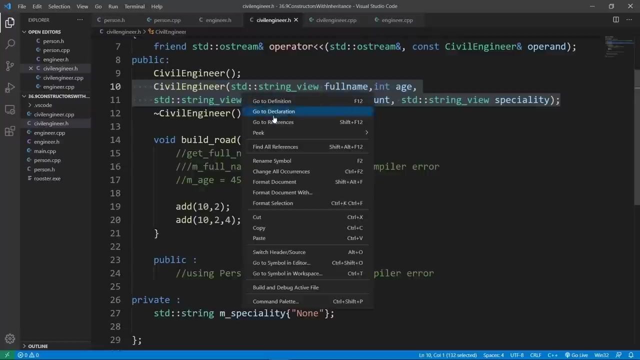 here and we're going to say speciality and we are going to put the implementation of this in our cpp file for a civil engineer. we're going to put this below our default constructor. let's grab this. i lost this somehow, so we're going to copy and we're going to paste down here. we're going to say that: 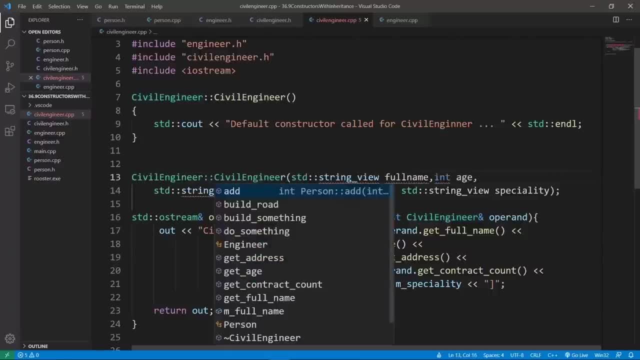 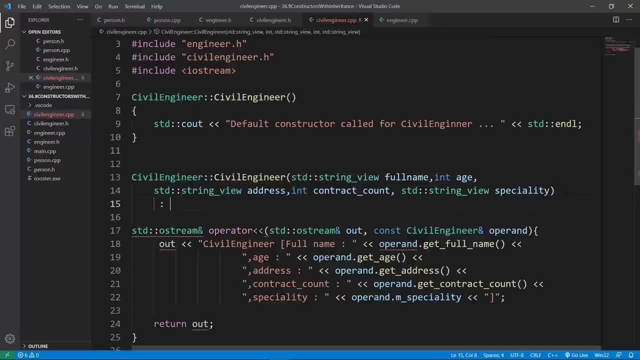 the contract count here belongs to the civil engineer class. we're going to use our scope resolution operator and after this we're going to put our initializer list in civil engineer. we will call our engineer constructor and it is going to be taken for effects. we're going to pass in the 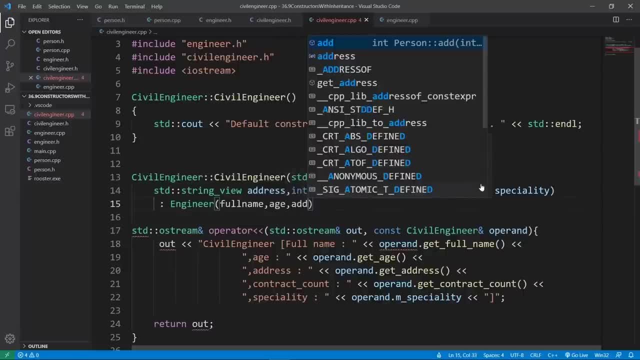 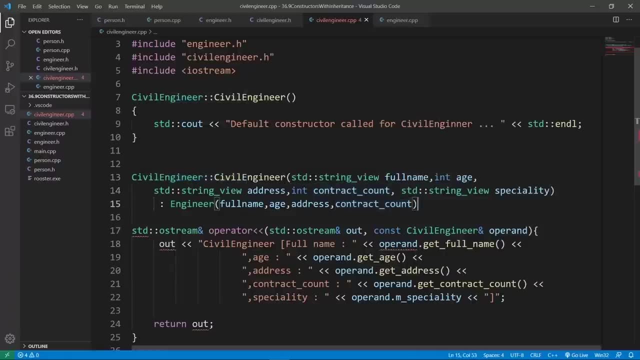 full name, we're going to pass in the age, we're going to pass in the address and we're going to pass in the contract count which we will get from our engineer. but we will also initialize our speciality member variable. so we're going to say: 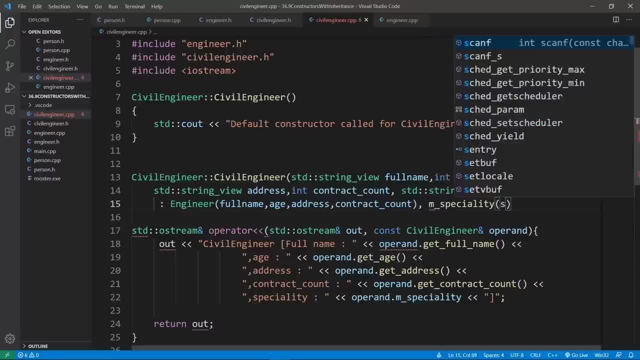 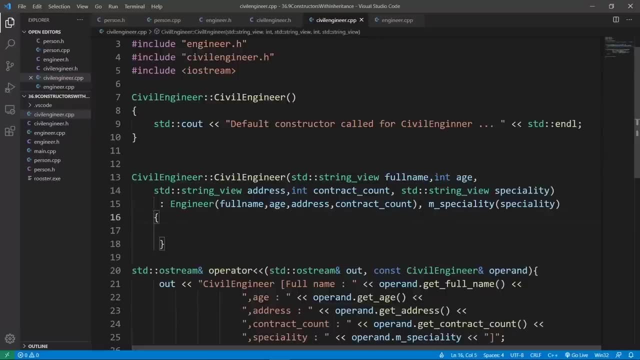 m speciality and we're going to pass the speciality information here and this is going to initialize our thing. we're going to put in an empty body and our information is going to be properly forwarded to our base classes. so if we build a civil engineer object, proper information is going to. 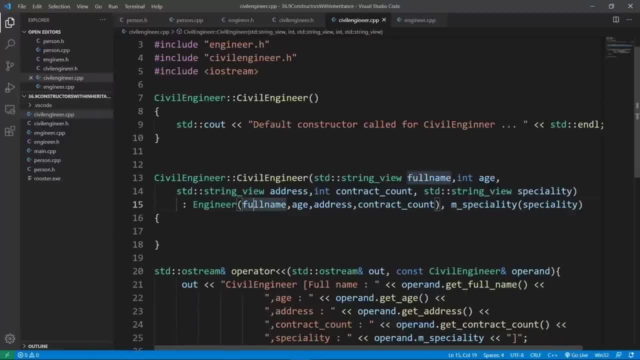 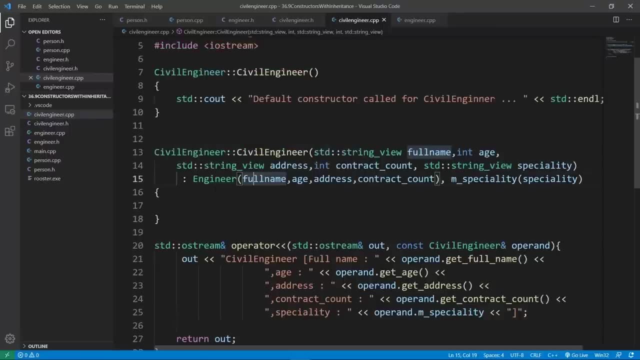 be forwarded to the engineer part of us and the proper information is going to be forwarded to the person part of us. now that we have this in place, we can put in our stdc out statements to let us know which constructor was actually called to build our thing. we're going to say that it was. 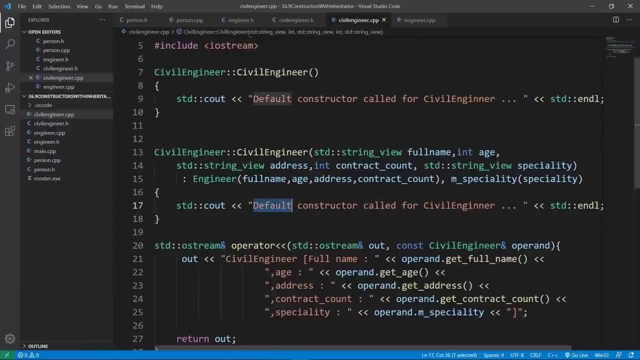 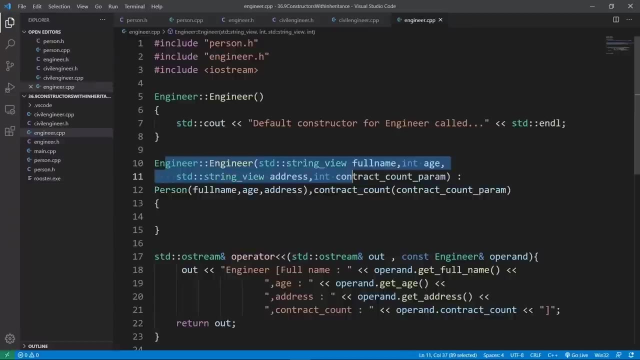 our custom constructor that was called. let's say that here we're going to say custom constructor, called for civil engineer. you are going to go to our engineer class and also say the same thing. let's go to the cpp file for that and we're going to put in our stdc out statement and we're going to say custom constructor. 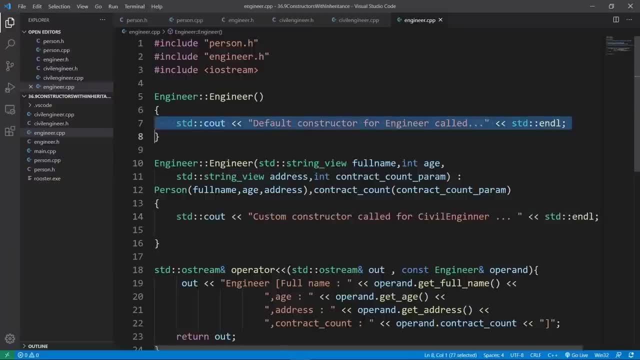 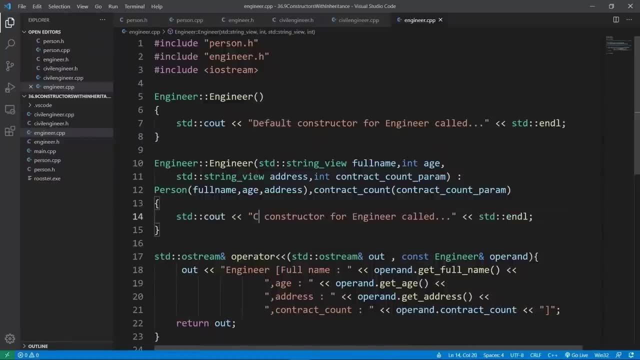 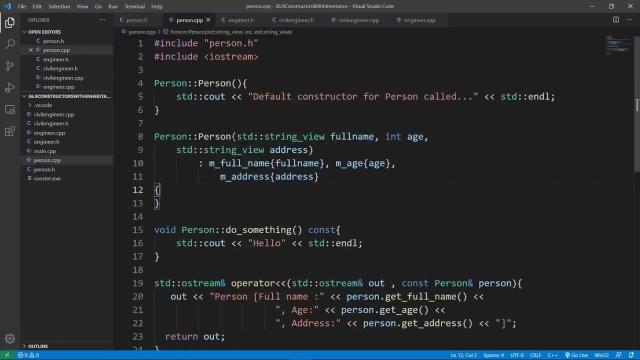 we can copy this to be consistent with what we had in our constructor- default constructor, i should say, and we're going to say: custom constructor called for our engineer class. we're going to go back to person and we're going to go to the implementation file and we're going to copy the message from our default constructor and 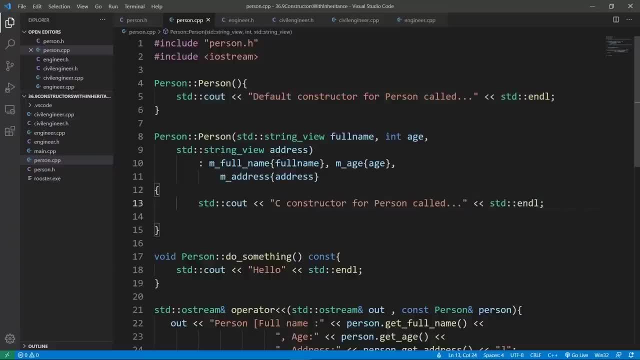 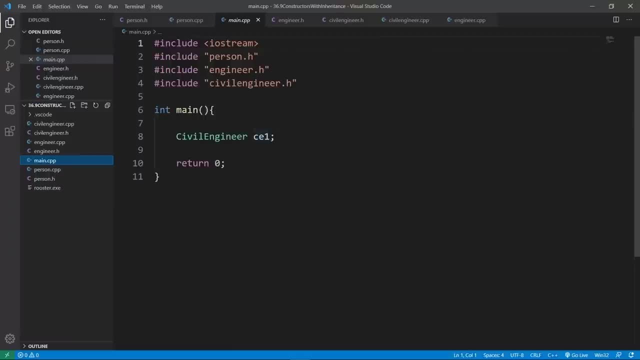 we're going to put this in and say that the custom constructor was called for person here. so now that we have these guys in, we can go to our main cpp file and include the classes. they are included here. we can try to create a person object just like we saw in the slides, and we're 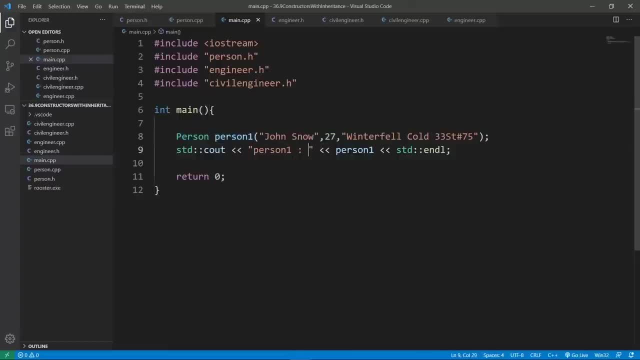 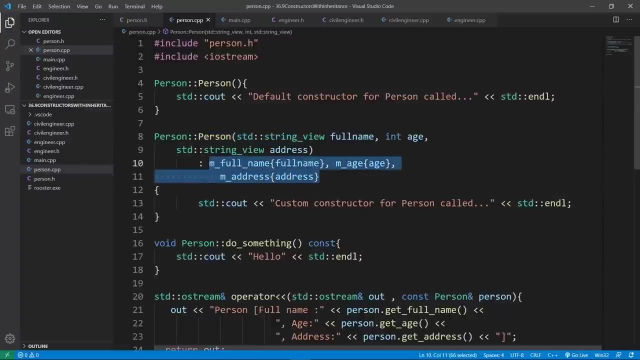 going to try and build this program and see which constructor is called to set up this person object. this shouldn't be rocket science. by now we know that our custom constructor is going to be called because we are passing three parameters which should be forwarded to our member variables. 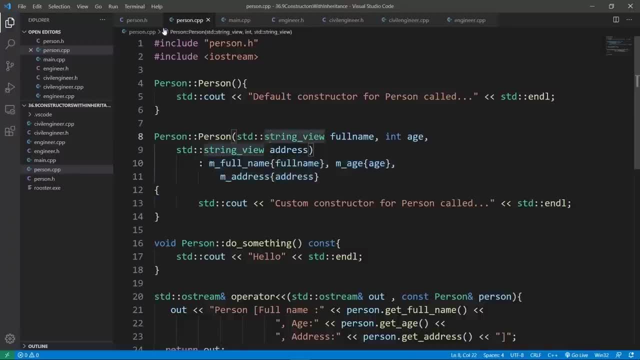 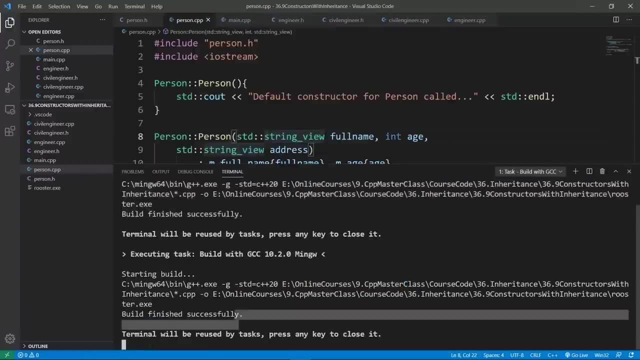 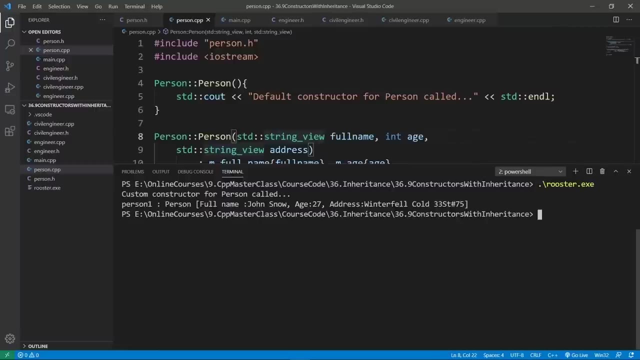 through this initializer last. so let's build with gcc and make sure this is what we expect. we're going to use our compiler here. the build is going to be good, as you see here, and if we bring up our powershell window and run rooster, we're going to see that our custom constructor is called. let's bring up the main cpp file so that. 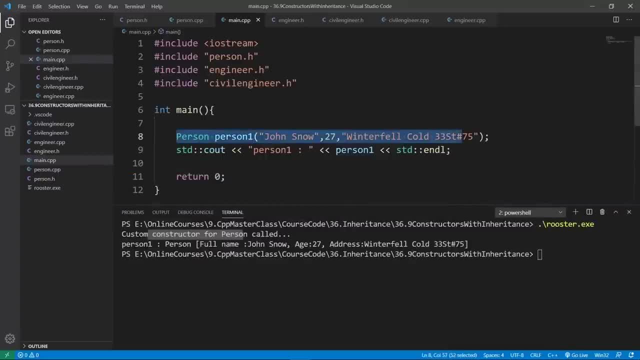 we can see our thang. we are passing this information here and we are printing our person object and we're going to see that the full name is jones snow, the age is 27 and the address is winterfell, cold and all this gibberish we have here. our constructor is really being called okay, so this? 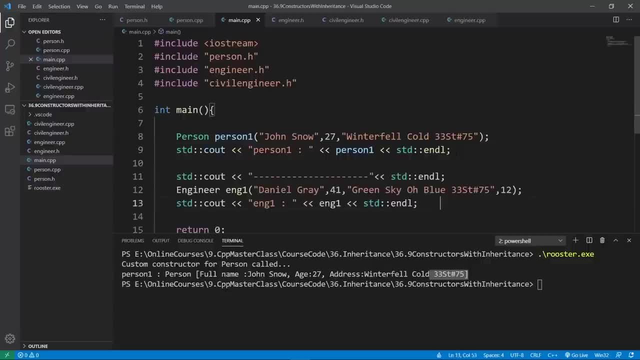 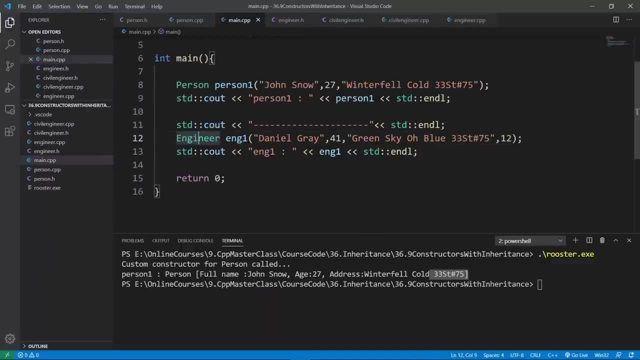 is working. we can also set up an engineer object and see that the information is being properly printed. and we can also set up an engineer object and see that the information is being plot, mostly propagated to the person port of our engineer object, because engineer is inheriting. 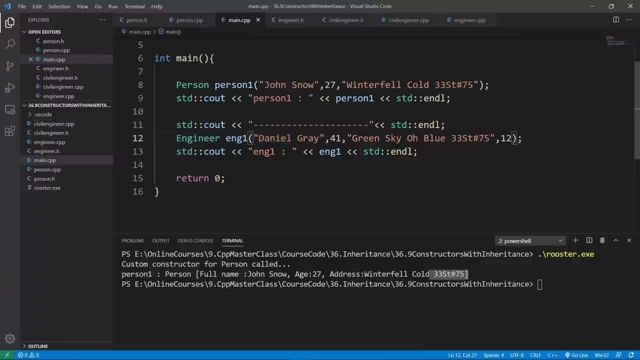 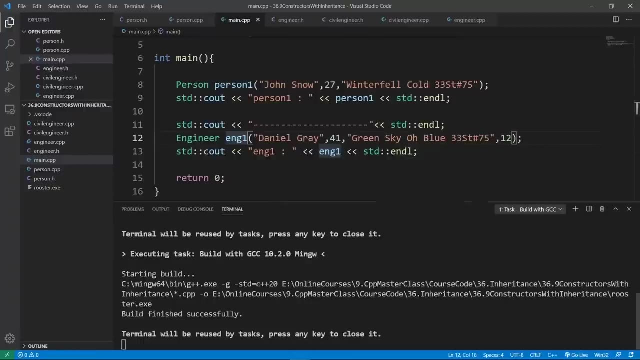 from person. we are passing the information for the full name, the age, the address, but we are also passing in the contract count which should be used to initialize the engineer part of us. so we are going to run the test world with gcc. the mult is going to go through successfully and we can bring 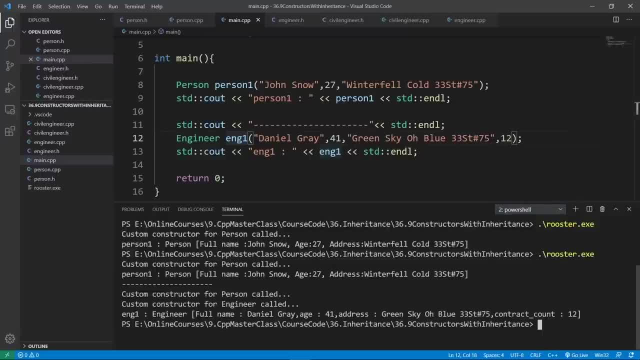 up our powershell window and let's see what happens next. now, if we have wender, so if we are going, we're going to run the same five minutes. so let's build this bcg the calls zehn control code, and we're and run the program again. we're going to see that we're going to print the. 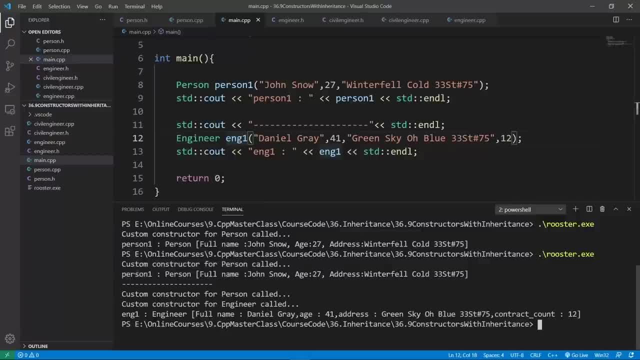 information for person: custom constructor for person called. but what we really are interested in here is seeing that the custom constructor for person is called for building our engineer object and then we call the engineer constructor, and again this falls in line with what we saw in the last lecture: the most base constructor is called first and then the most. 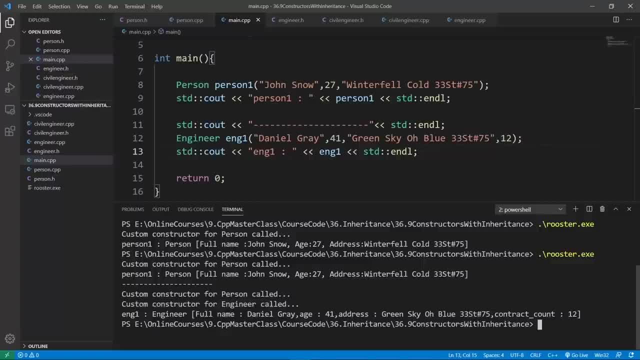 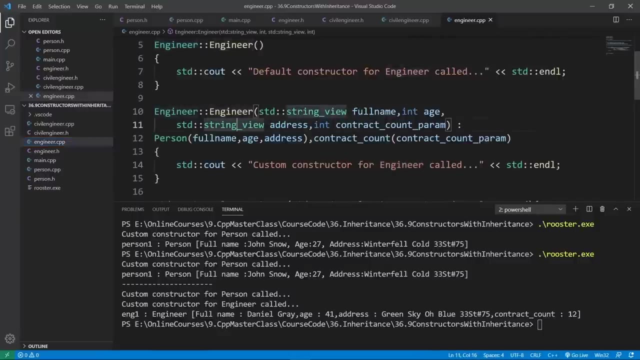 specialized constructor is called last. in this case, we are just setting up things in such a way that our custom constructors are called and we do that from our engineer class by calling the base constructor explicitly using the syntax that we have here in our initializer list after we have the base. 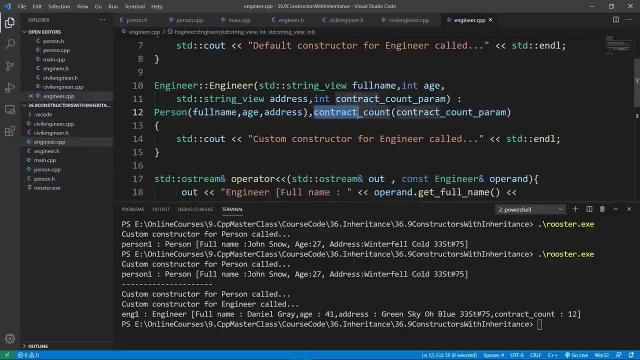 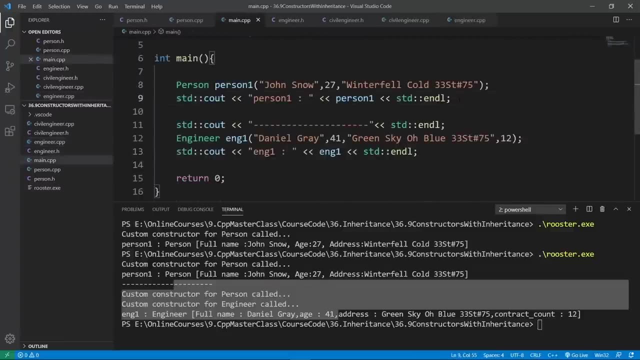 constructor called. we are going to initialize our own member variables and that's what we see, and in this way, the information for the current class will be initialized properly, and this is what we see here. I think this is a little bit misleading, because we still have the information from the person objects that we will print it out here. 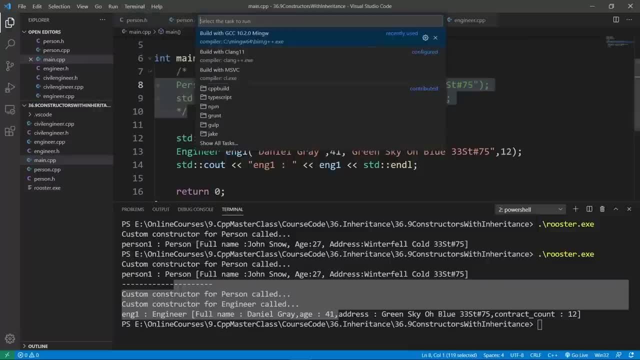 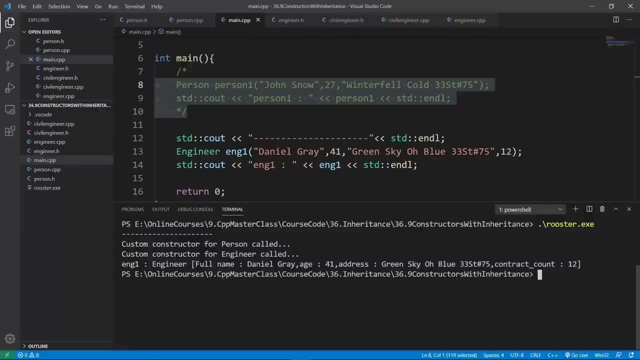 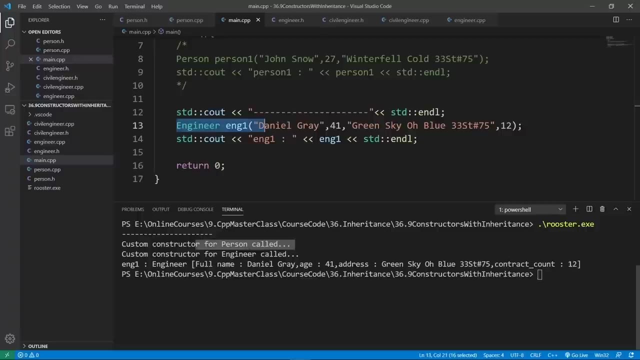 we can comment this out and build again. we're going to pass this through GCC to build our program. the world is going to be good. we can clear, clear and run rooster and we're going to see that the custom constructor is called for a person to set up the person part of us and then another layer of. 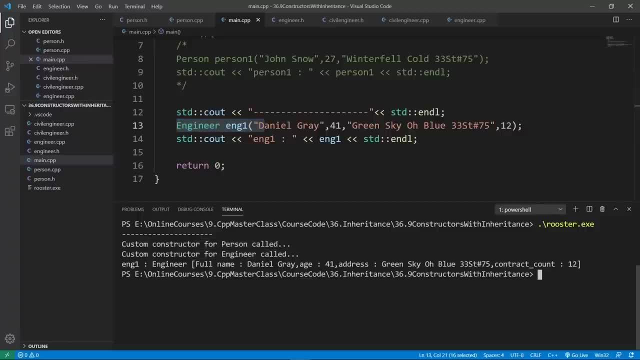 engineer is going to be set up in our object to initialize the contract count member variable part of us and we're going to have the information here. so if we print the full name, we're going to get Daniel gray. the age is going to be 41, the address is going to be the gibberish we expect here and the 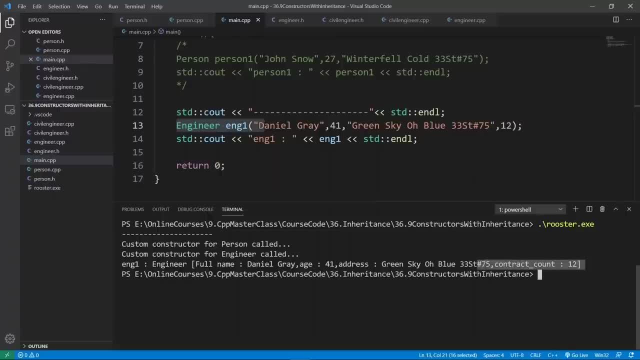 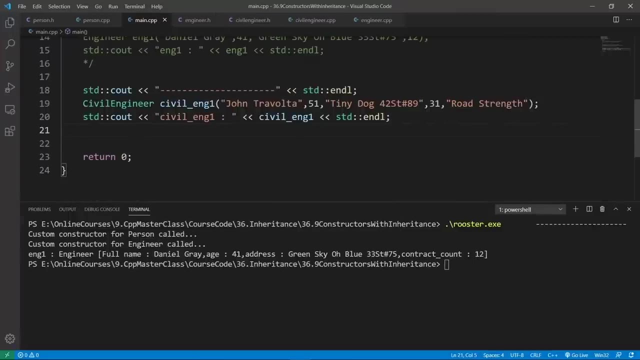 contract count is going to be passed in successfully and then we're going to create a civil engineer object. and this is really cool. we can also comment this out and set up a civil engineer object. we can do that, okay, so let's go down and put this in place. we're going to create a civil engineer object. we can close up. 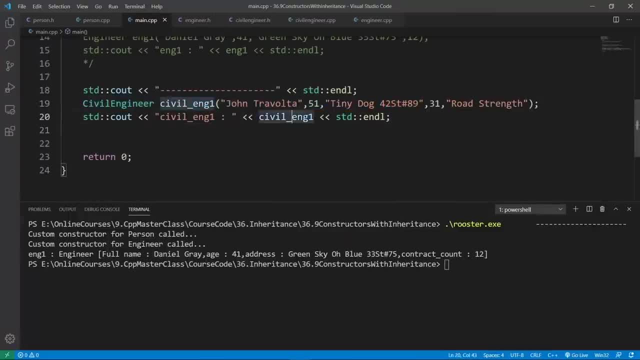 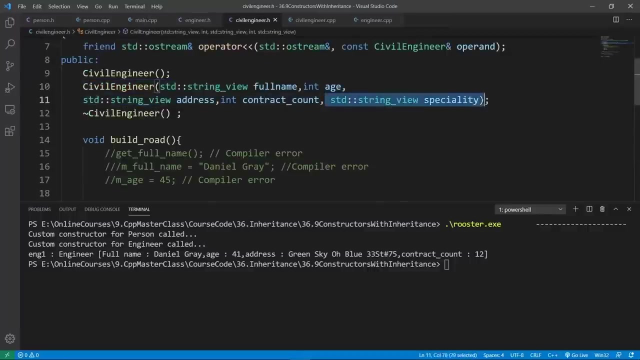 the left side bar here to have some more breathing room. we're going to build a civil engineer object. we're going to pass in full name, age, address, contract count and a speciality which I think we expect from our civil engineer: custom constructor. here that's going to be an STD strength. 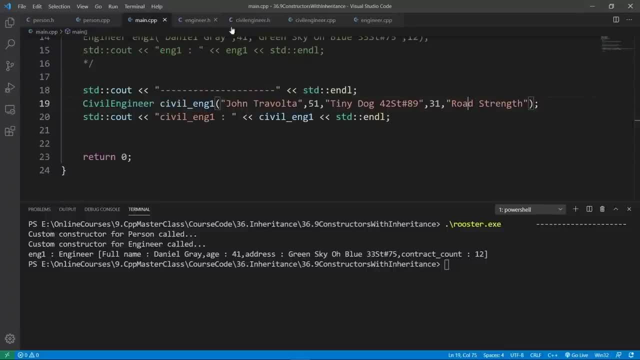 that's what we are passing in here. I should say that's going to be a string view, but we can pass in string data, just like this, and the string view is going to take it. so what we're going to see here, we're going to see the person. 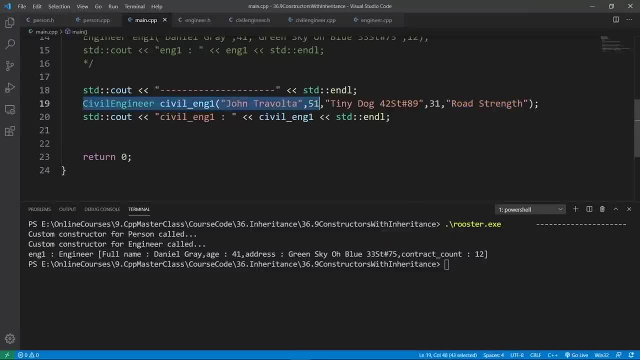 constructor called the person custom constructor, I should say we're going to see the engineer custom constructor called and after that we're going to see the civil engineer custom constructor called to pass and forward all this information in related parts of our civil engineer object. let's build and see. 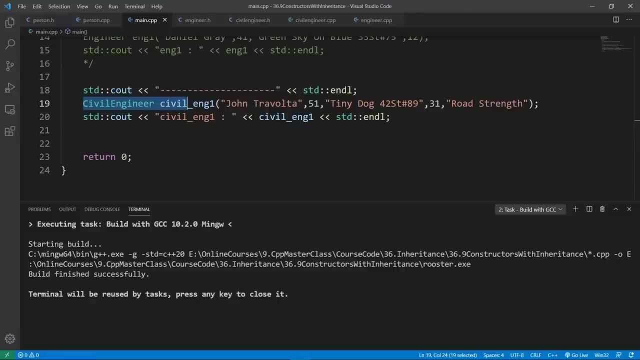 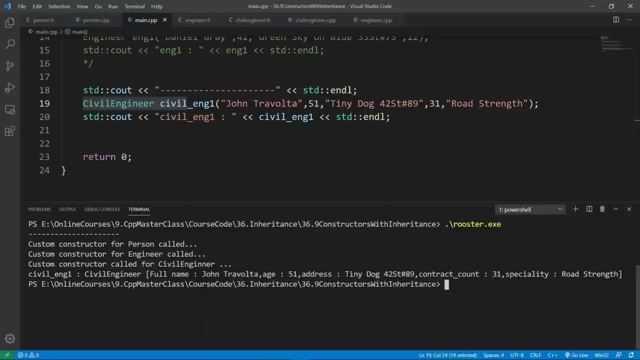 that this is actually going to even compile. the world is going to be good. we can clear and run rooster, and we're going to see that this is exactly what we expect. the custom constructor for a person is going to be called. after that, the custom constructor for engineer is going to be called. 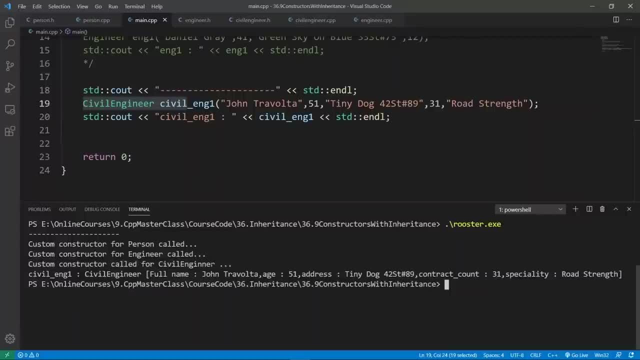 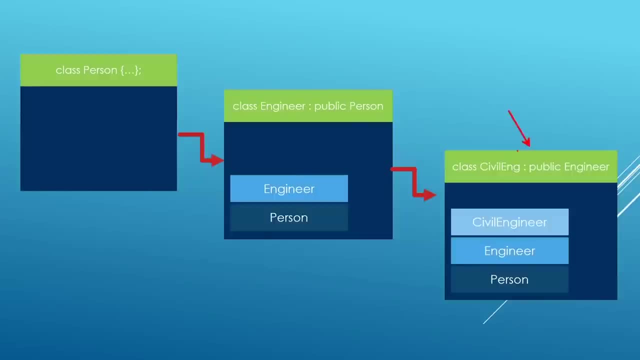 then the custom constructor for a civil engineer is going to be called, and this really falls in line with what we expect if we are building a civil engineer object and the civil engineer class happens to be inheriting both from engineer and from person. we're going to have the person part. 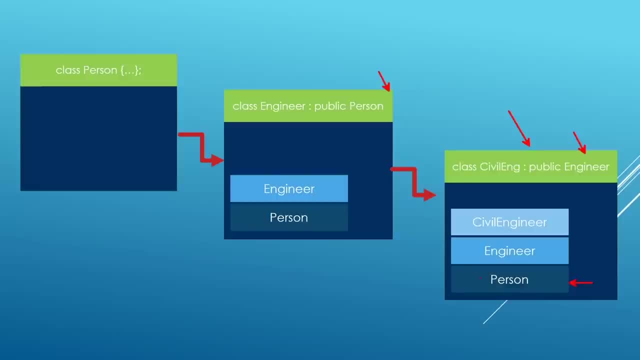 of us built first and because of this we're going to see the person constructor called. but in this lecture, the real focus is getting our custom constructor called. so the person custom constructor is going to be called. after that we're going to call the custom constructor for. 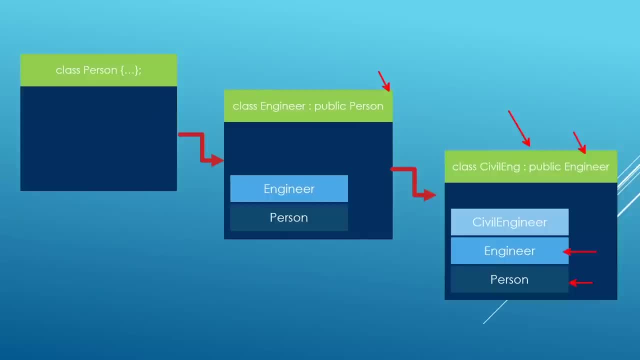 the engineer part of us and that's going to set up the engineer specific member variables in our object. after that we're going to set up another layer of civil engineer in our object and this is going to initialize the member variable that belonged to the civil engineer part of us in. 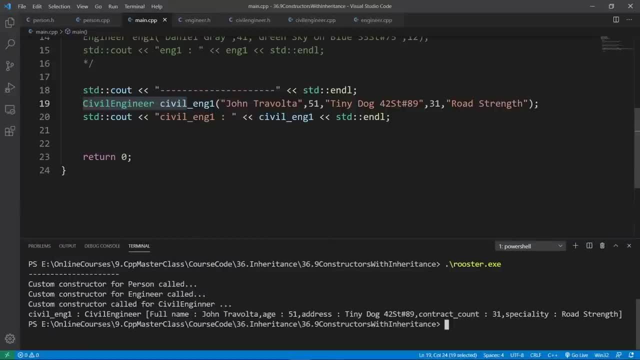 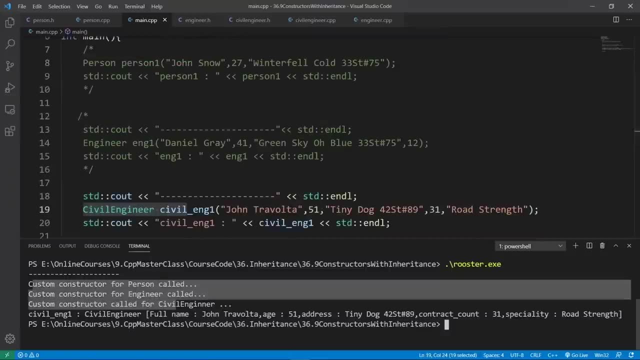 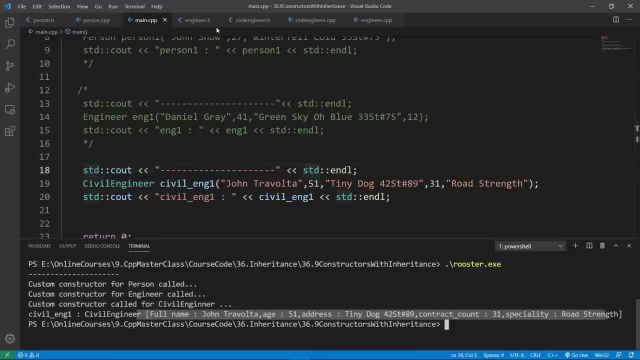 our object. so this is really the main goal in this lecture: showing you that you can set up things in such a way that your custom constructors are called when setting up your object in layers, as you see here. okay, now that we have this working, i want you to see that there are some bad ways to. 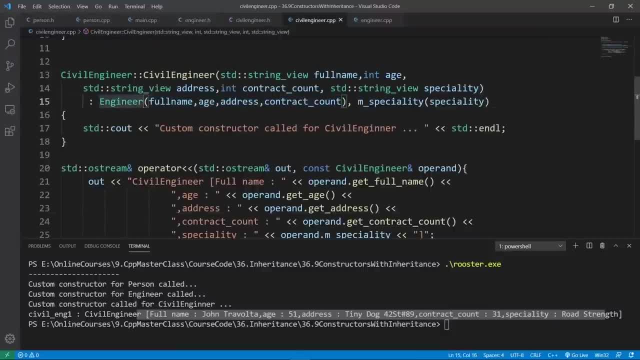 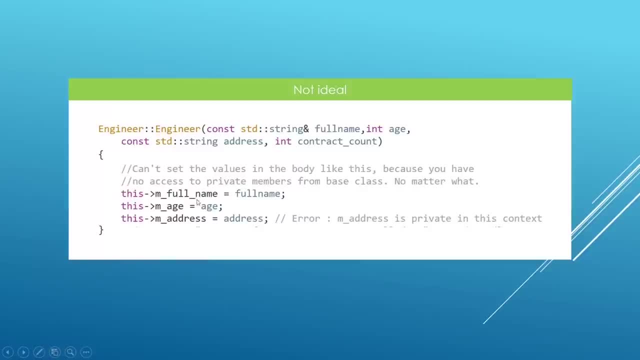 do these things and some people are actually going to try to set things up in that way. the first bad way is to try and initialize our custom constructor for the civil engineer part of us and that's going to be our member variables in the body of the class. if you do things like this again, this is 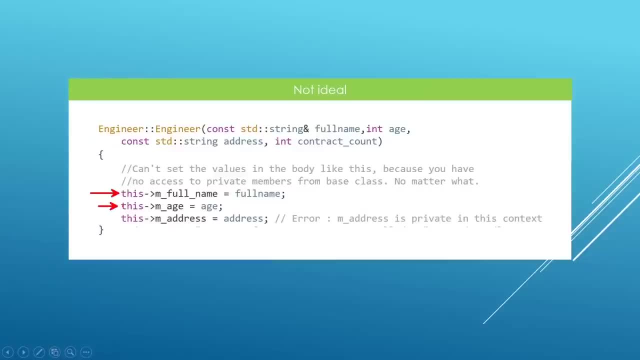 going to work because full name and age are going to be inherited publicly from the person class. so the code here is going to work. but we have no way to initialize the address member variable because it is private to the person class. so if we try to access that we're going to get a compiler error. 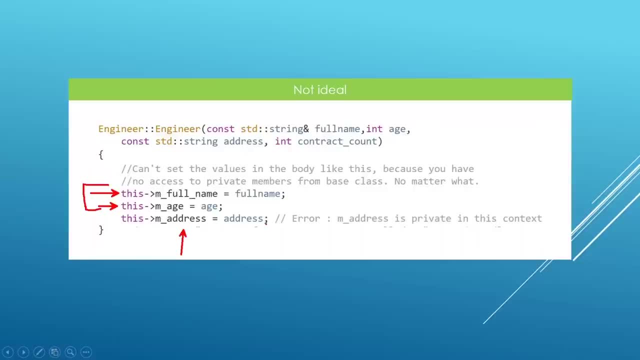 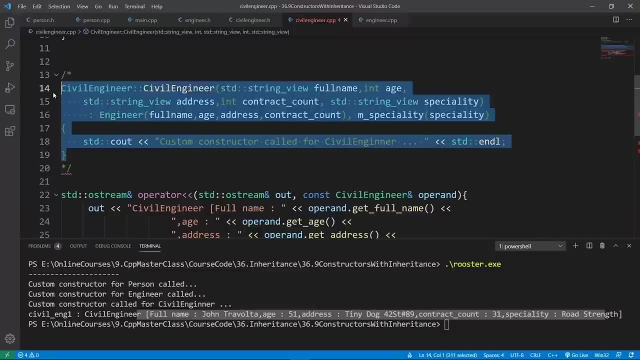 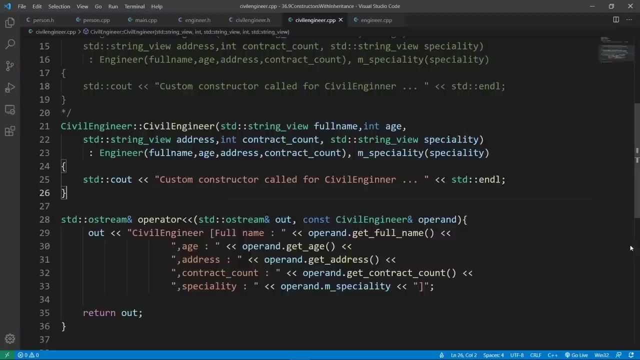 let's try this out in code and see the actual compiler error. to try this out, I am going to comment out the good code here and I am going to copy and put in something that is going to be problematic as we saw in the slides I am going to paste in my constructor here. I should close my PowerShell. 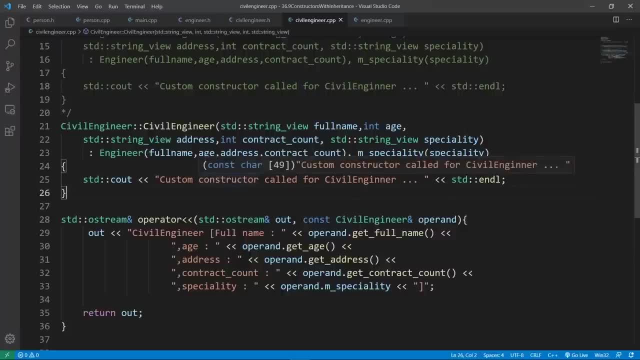 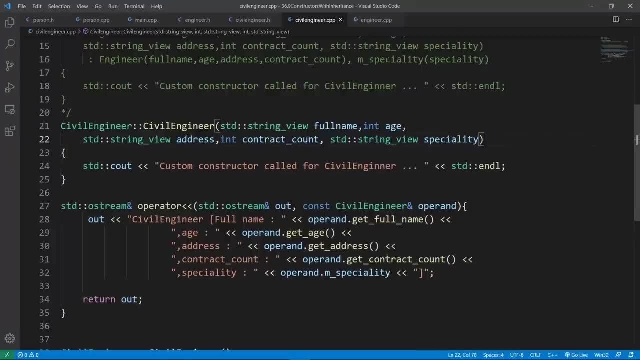 window here and I am going to take out my initializer list because we're not going to be using that here and we're going to just grab the data and use that to initialize our data in our member variable here. so we're going to grab the full name and say mful name. 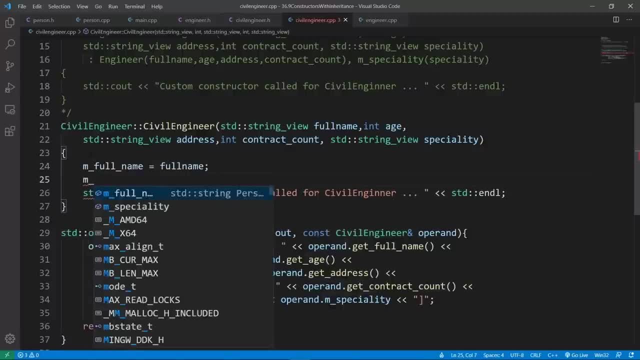 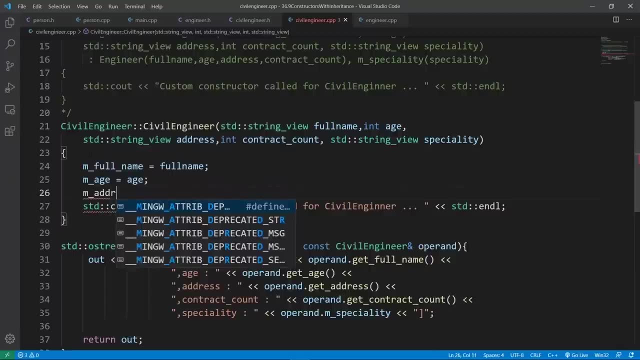 equals full name. we can do that. we're going to say mh equals age. that's the information we get. we're going to say m address and you see that we don't even have that in autocomplete. so we're going to pass the address. we're going to be stubborn and ignore these squiggly lines and 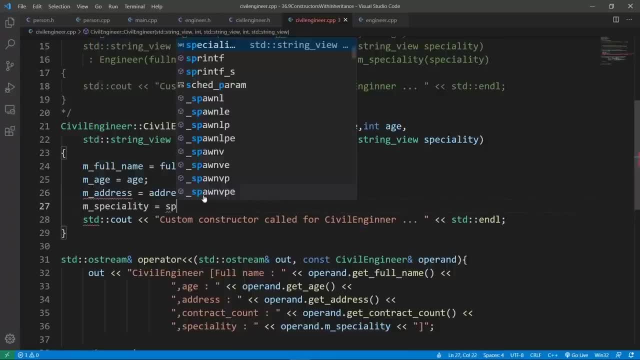 we're going to say m speciality and we're going to grab this speciality and pass that end. but you see that line 26 has a bunch of squiggly lines. the reason is the m address member variable is invisible and not manipulable from our civil. 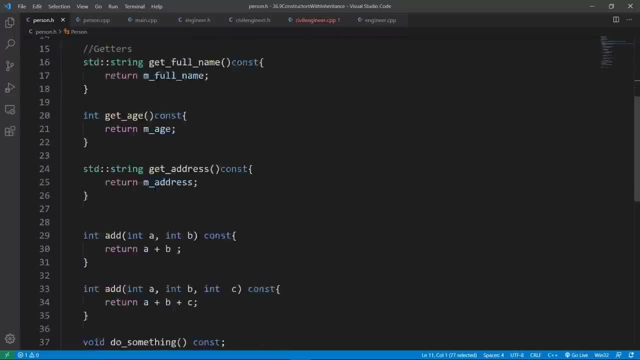 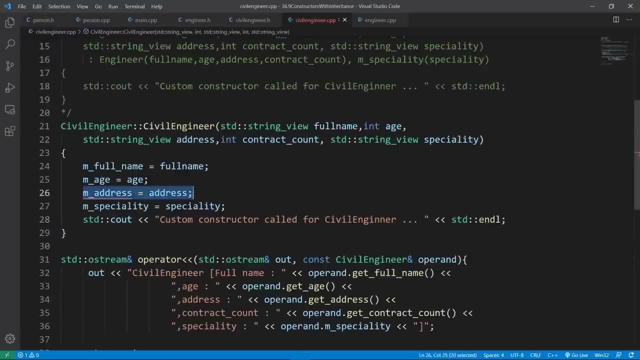 engineer class. again, the reason is that the address member variable is private to the person class, so the civil engineer class has no business initializing this in the body. this is not going to work. so if we try and the world this, we're going to pass this through gcc. we are going to see that. 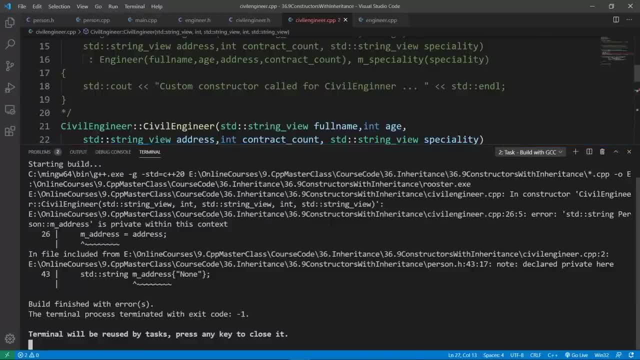 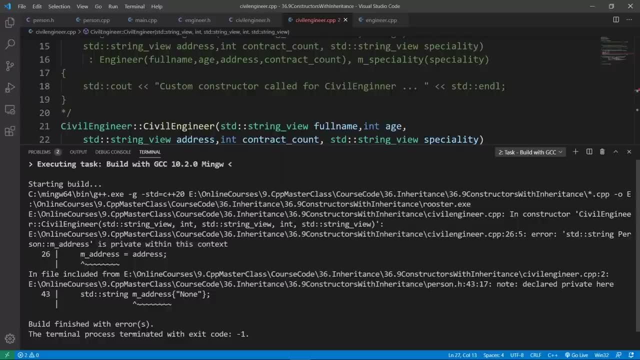 the world is going to finish with errors and if we go up we're going to probably see the error person m address is private within this context and we have no business accessing that in the civil engineer cpp file at line 26.. this is what we see. 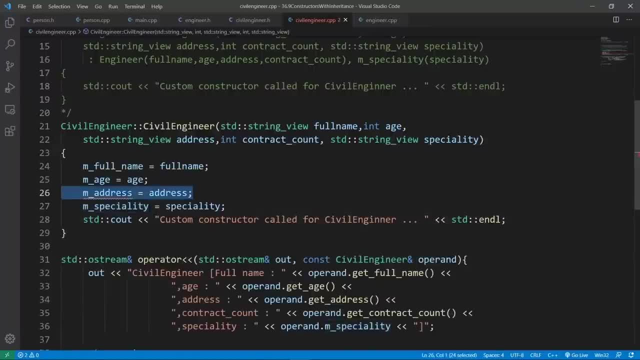 here, and this is the offending line. we shouldn't really be doing this. if we comment out this line, this is going to work, but our member variable is going to be left with a junk value, and this is really not good, because our address- we worked so hard to set up in our parameter here- is just going to be ignored. so this is bad. 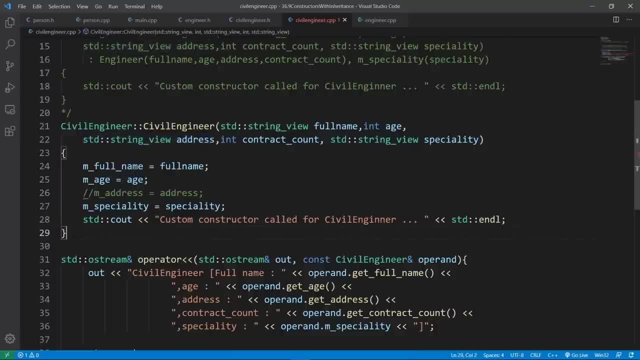 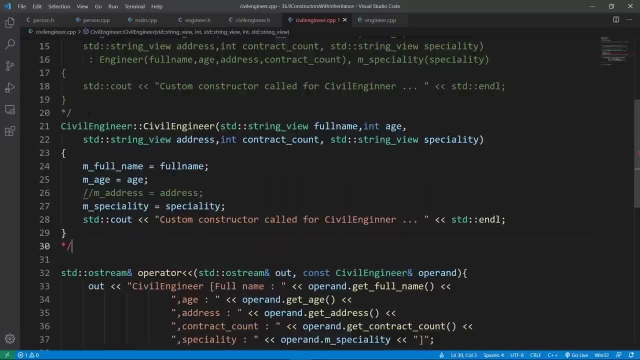 you shouldn't really be initializing your member variables like this, especially if you have an inheritance hierarchy in your classes. so we're going to comment this out and say that this is really bad. it's going to give you compiler errors and some of you are going to say, okay, this is not. 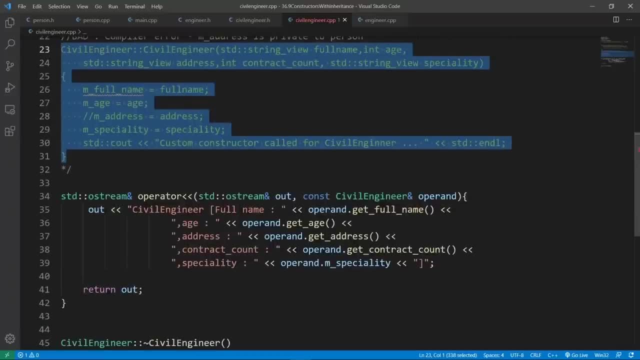 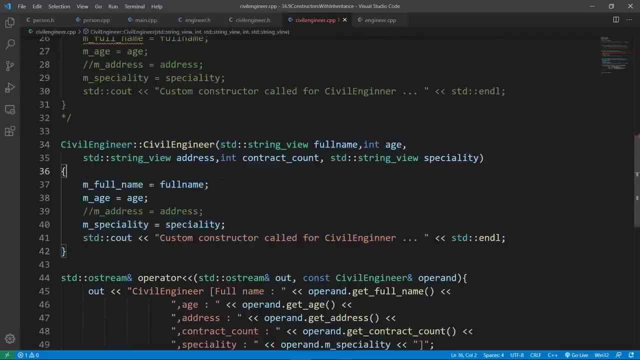 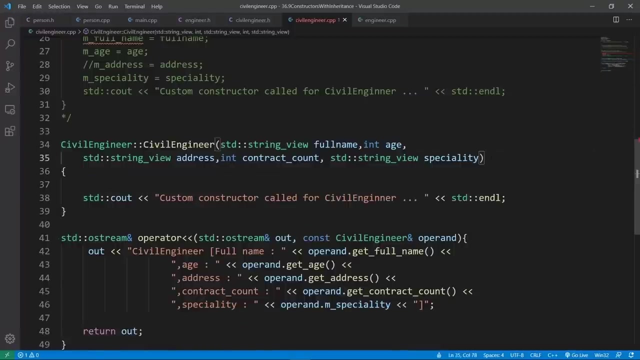 working. but what if we try to use an initializer list directly? let's see if that actually works. we are going to set up another constructor here and we are going to set up the data in our initializer list. we're going to say, let's say m full name and pass in the full name. we can do that. 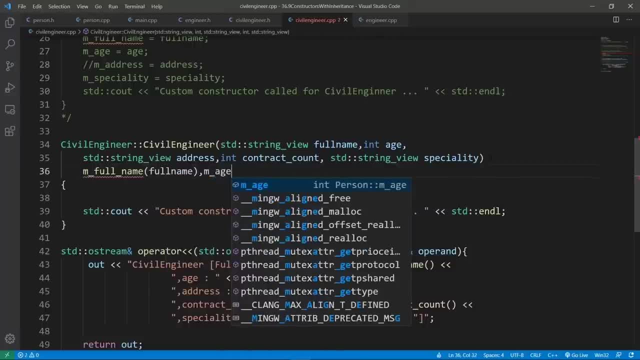 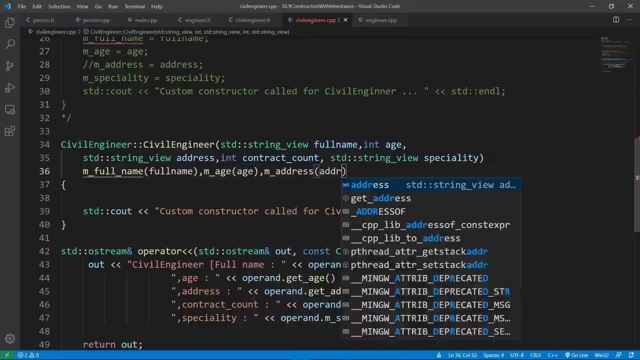 let's try this out. we're going to say mh and we're going to pass age- we can do that- and we're going to grab the address and we're going to pass an address here and after that we're going to say m, speciality a. 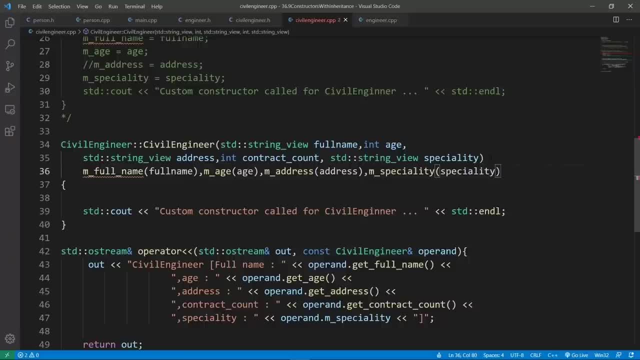 to pass in our speciality information. what if we do something like this? but you're going to see that we have squiggly lines here, and the problem with this way of doing things is that the civil engineer class has no business initializing things that belong to the person. 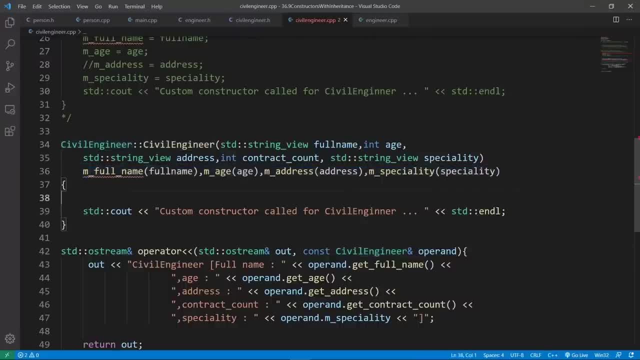 class in the initializer list. your initializer list only has the capability to initialize the member variables that belong to the current class, and m- full name, m h and m- address don't belong to the civil engineer class. that's why we're going to have a compiler error if we try to set up things. 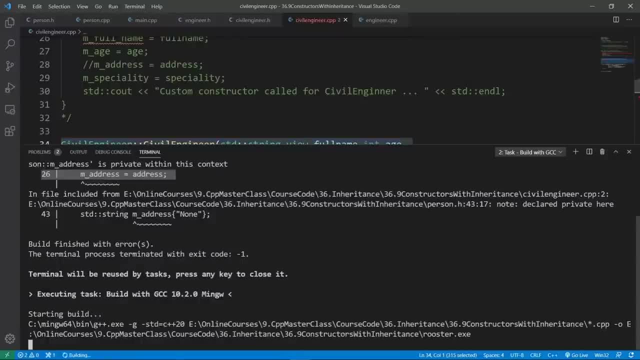 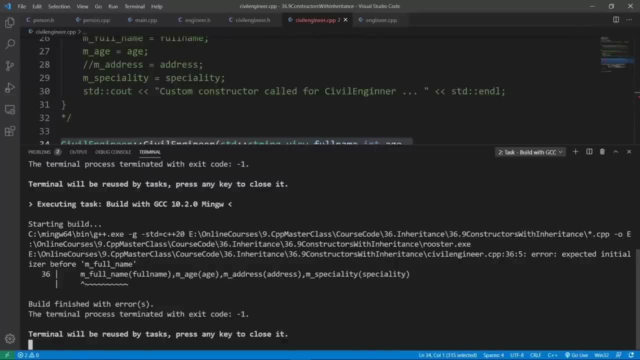 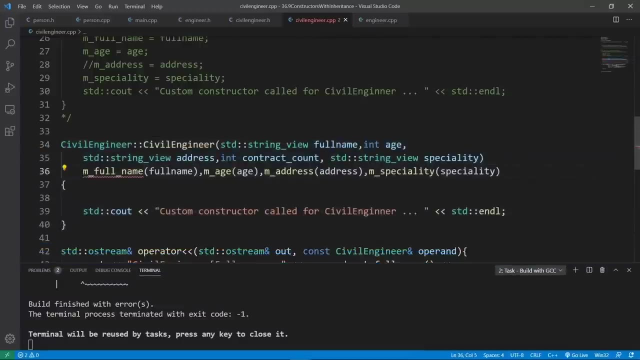 in this way, if we're trying to build the program, we're going to get a weird compiler error. we're going to see that the build is going to finish with errors and it is going to say expected initializer before m- full name, and we need a colon, colon here. sorry for this. so this is not the error we expect. but you see, 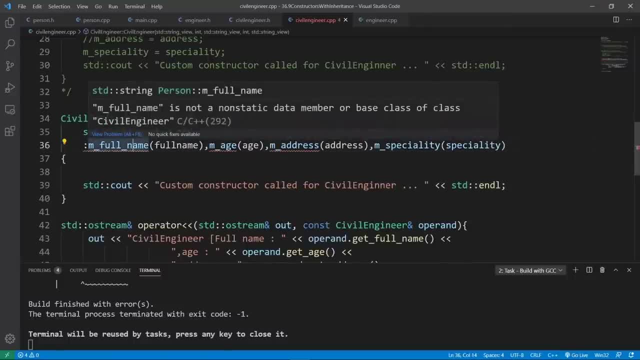 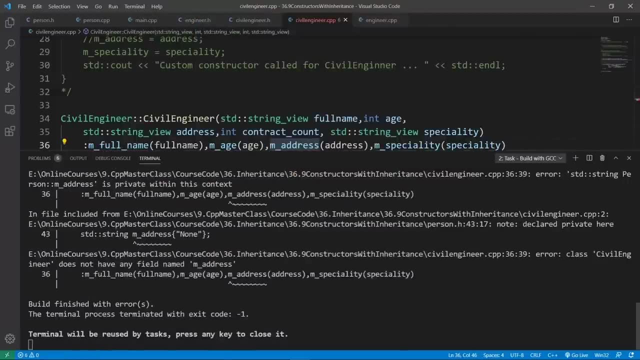 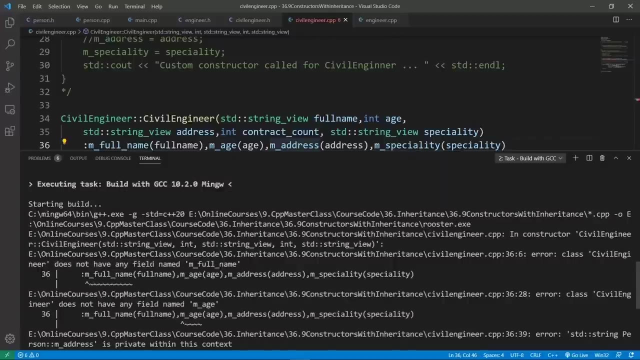 that the moment we do this, we have a bunch of squiggly lines on full name, age and address and let's build and see the problem we have and we're going to build with errors, as we see here. if we go up, we are going to see our errors. civil engineer does not have any field called. 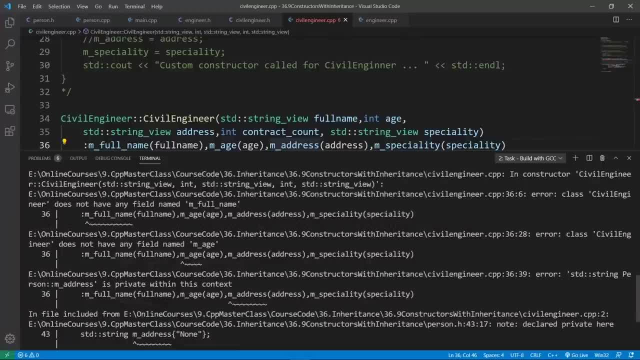 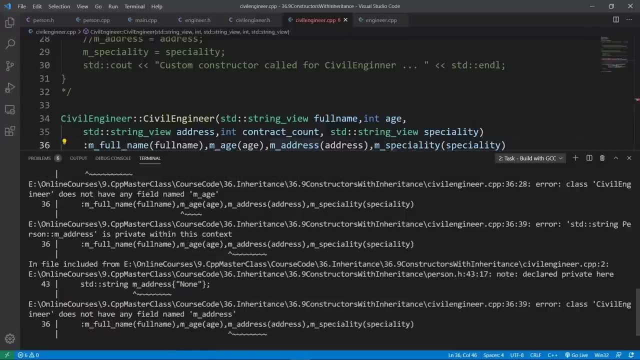 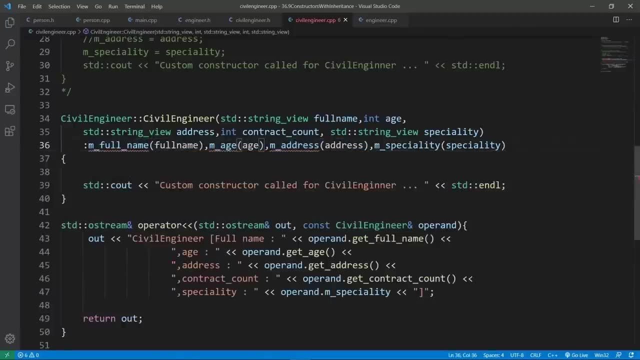 m full name. we're going to see that civil engineer doesn't have any field called m h and civil engineer doesn't have any field named m full name or m address here. that's the problem. we have no business initializing these member variables that don't belong to the civil engineer. 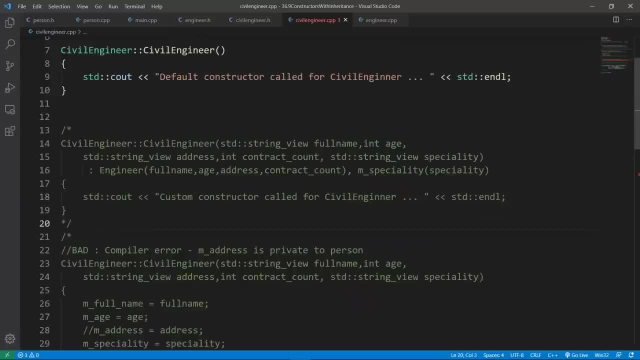 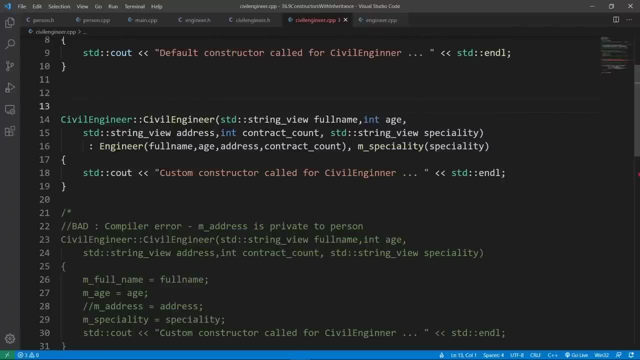 class in the first place. so this is also not going to work. the best bet we have really is to call the base constructor and let that initialize the member variables that belong to our upstream class in the inheritance hierarchy. from here we have the best constructor, which is our member variables, and 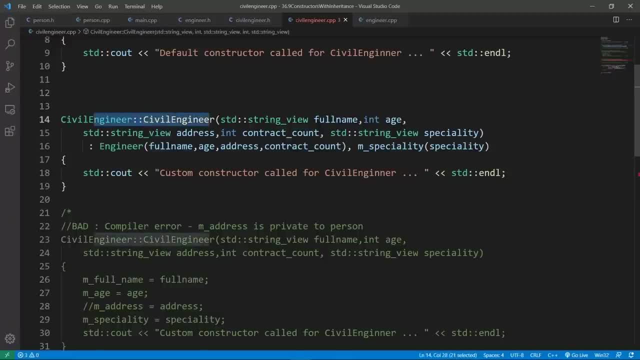 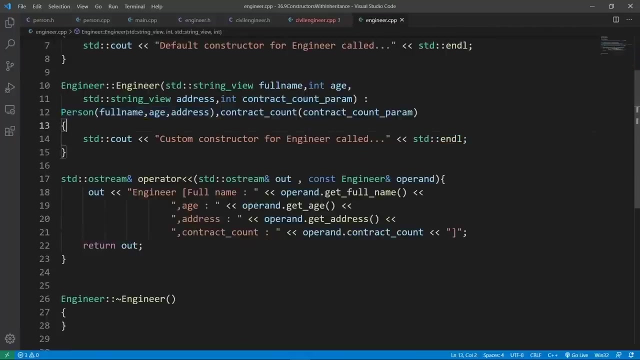 For example, in our civil engineer constructor. here we need to call the engineer constructor to initialize the engineer part of us And we're going to be forwarding the information: the full name, the age, the address and the contract count. The engineer class is in turn going to call its base constructor to forward the information. 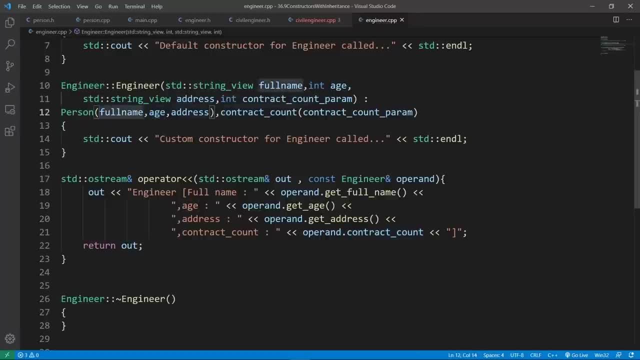 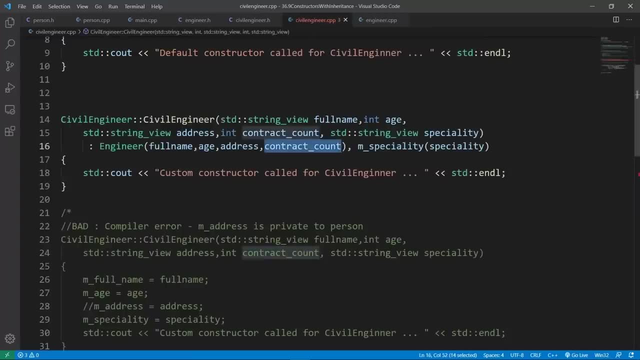 about the full name, the age and the address And it is going to initialize its own member variable, mContractCount, And the information is going to be passed in correctly And if we're trying to build our class now, we're going to see that everything is going. 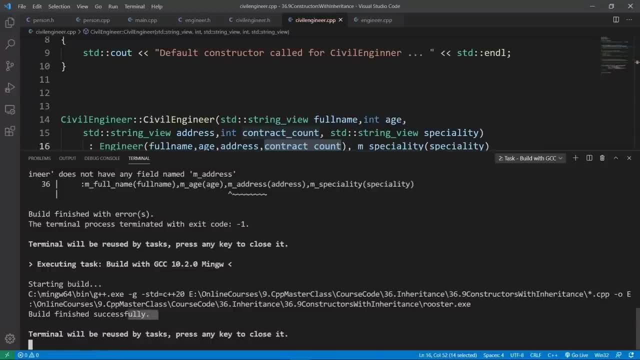 to work, And I really wanted you to be aware of this, because the moment you understand this, you're going to set up your inheritance hierarchies in a way that is going to make sense And you're not going to be getting all these weird compiler errors. 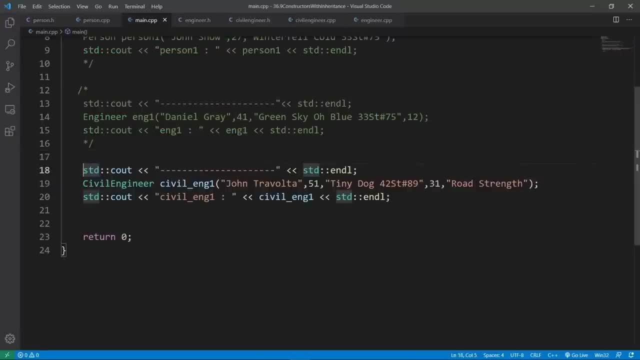 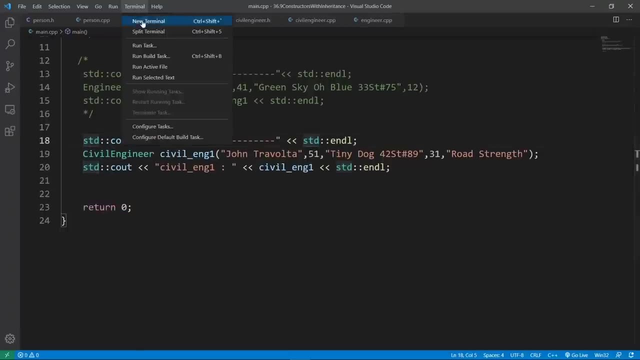 This is really all we set out to do in this lecture: showing you how you can set up your own custom constructors in your own inheritance, And at the moment you do that, you're going to get your classes called in the order that you expect. 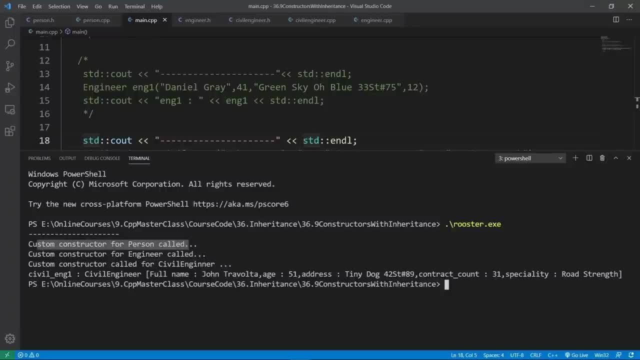 Things are going to be set up in layers. The base constructors are going to be called in a way that you expect And your objects are going to be built in a way that you can print them and see the information that you expect set up in your object. 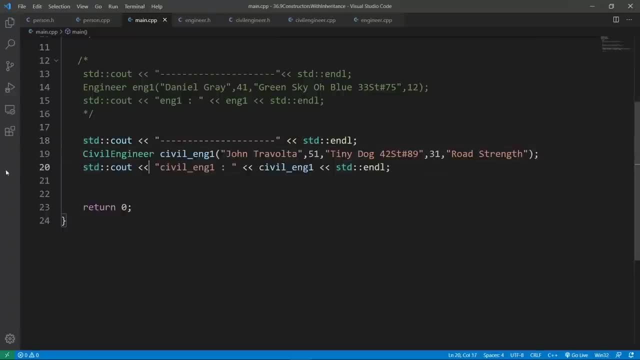 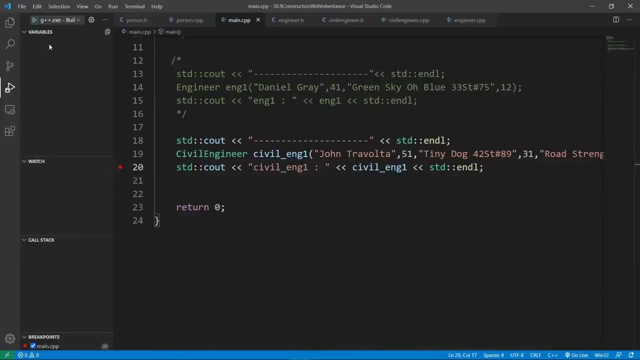 If you want, you can also use a debugger to see the information in your thing. So we're going to set up a breakpoint here And we're going to bring up Our debugging tab. We're going to hit the green button to start debugging this program. 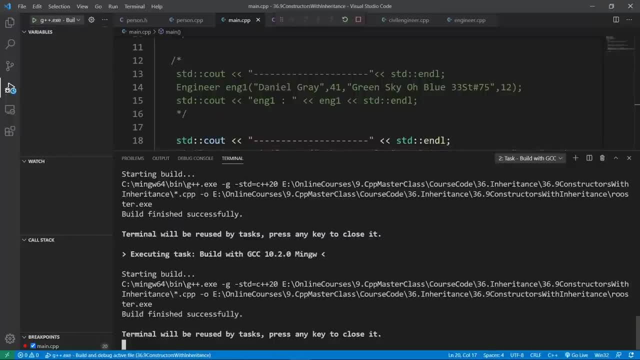 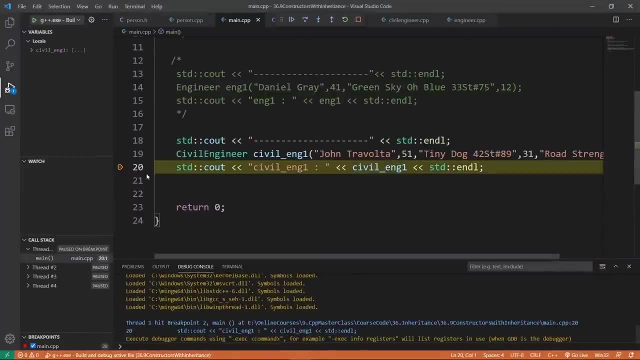 The binary is going to be set up. Once the build is good, the binary is going to be passed in our debugger And we are going to hit our breakpoint in a minute. Let's wait for this. So we have hit the breakpoint at line 20.. 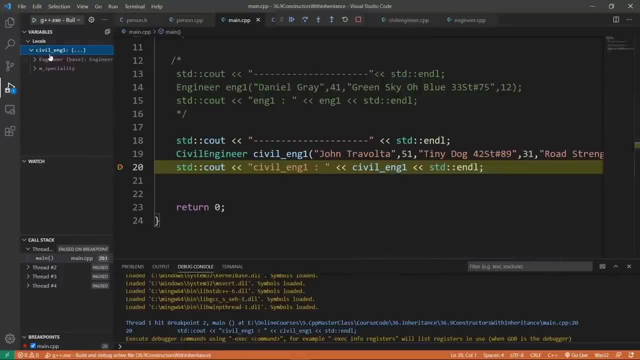 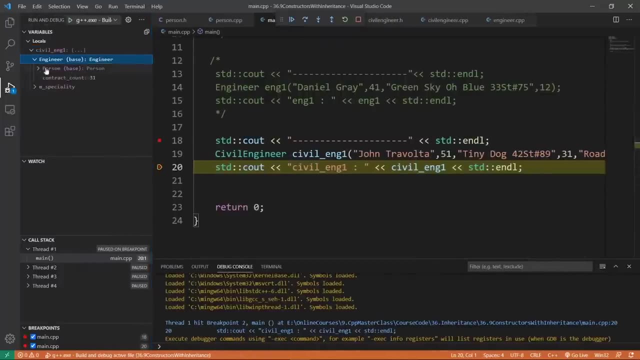 And if we expand our civil engineer object in our locals, we're going to see that we have an engineer part of us. We can expand that And see that we also have a person part of us. If we look at person, we're going to see that the full name is 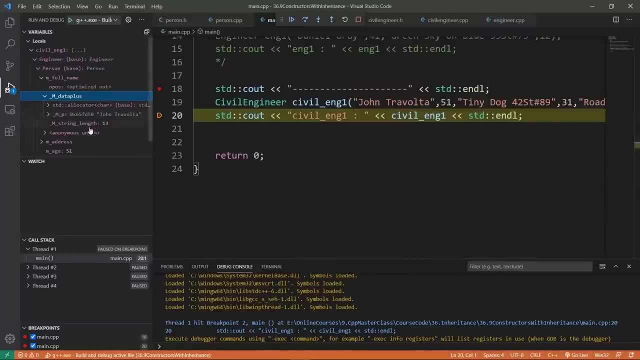 We can see John Travolta, which is what we are passing here. We can also look at our age. The age is 51, as you see here, And we're going to also have information about our address. If we expand this, we're going to see that the address is this gibberish that we just put in. 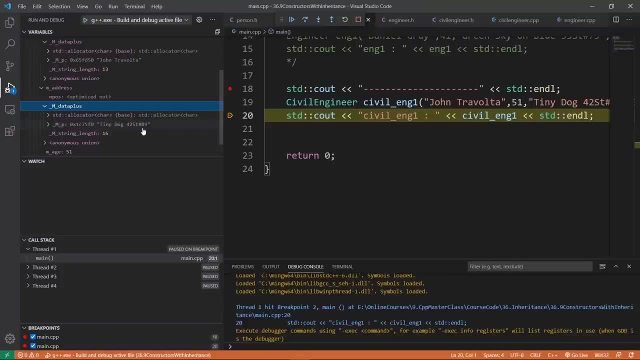 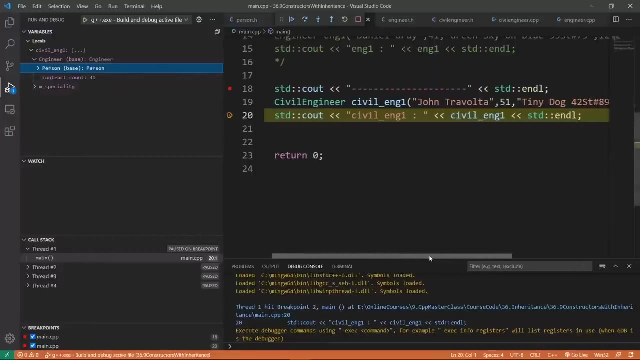 Tiny dog, 42 straight and a number 89. We can see this information here and you can really expand and see all these things that make up our object. For example, we can see the information about the contract count, which is 31,, and it is what we are passing when we 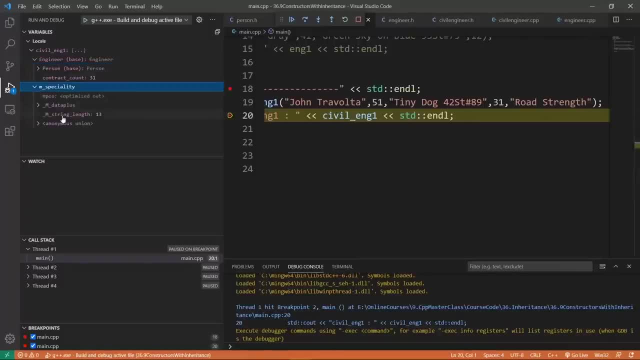 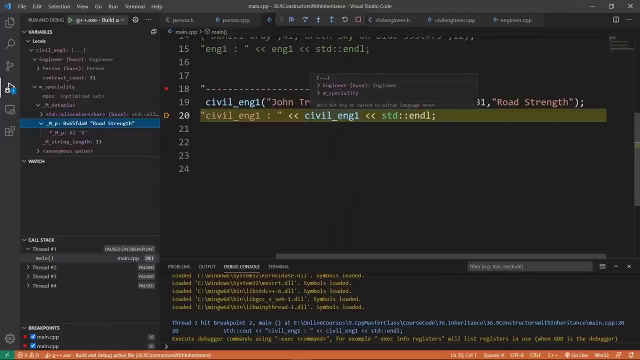 built this object here And the speciality happens to be Roger's strength, as we see in our locals. here You can really see all these things. we are going to stop here in this lecture and the next one We're going to explore how copy constructors work in our inheritance hierarchy. 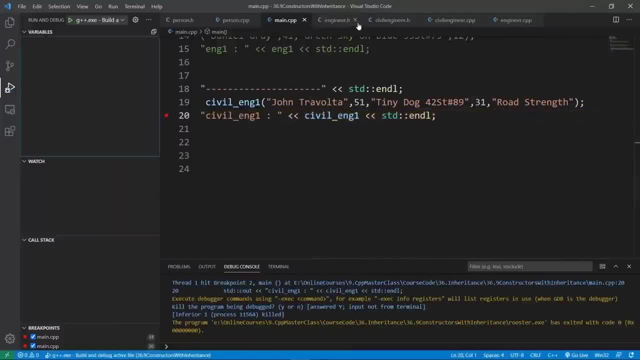 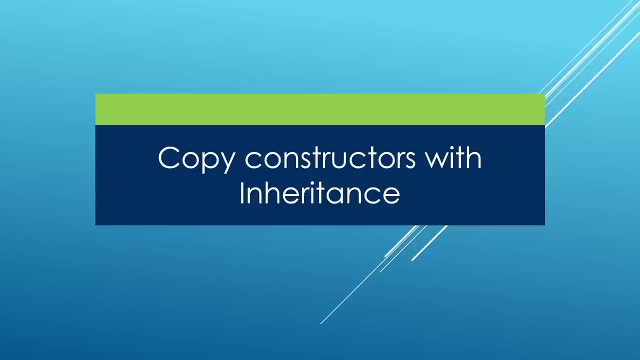 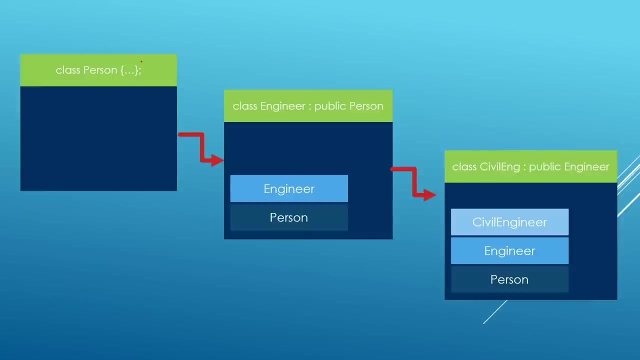 So go ahead and finish up here and meet me there. in this lecture, We want to explore how copy constructors work with our inheritance hierarchies, and we will still be using the same example we have been using in this chapter. We will have this inheritance hierarchy and we will still be using the same example we have been using in this chapter. 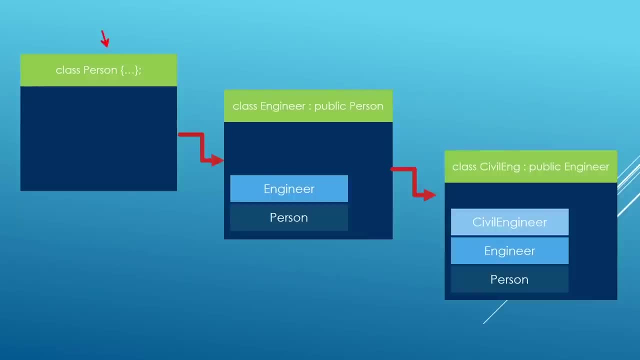 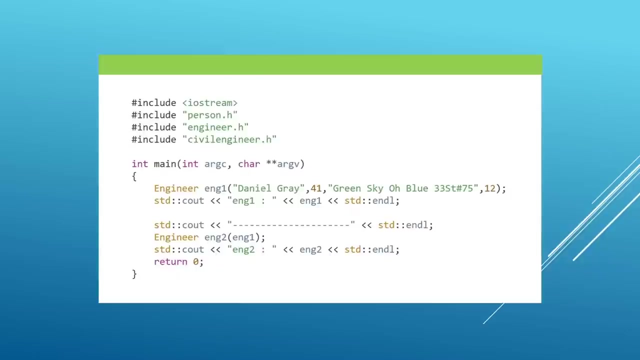 The base class is going to be person related to be inherited from that publicly to create an engineer class, and we will be inheriting from the engineer class publicly to create the civil engineer class And with this we want to be able to copy, construct objects and the code we want to be running is something like this: 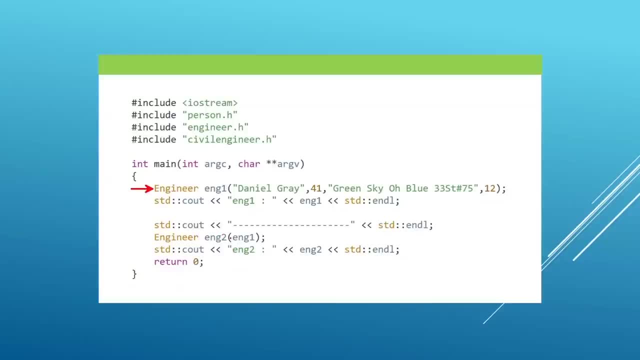 We have an engineer object. We want to be able to create another object from this engineer object using the syntax here And from what we already know. This is going to call our copy constructor. The funny thing is, this is going to work by default, even if you don't put in your copy constructor. 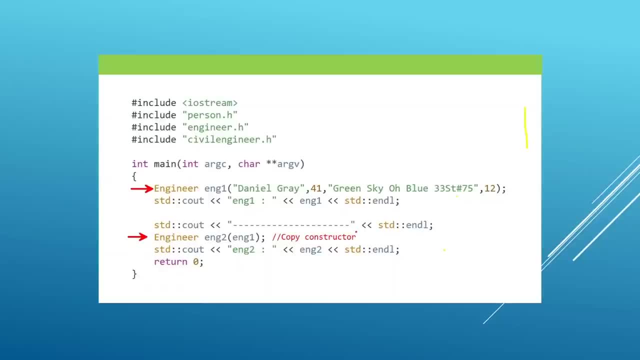 The reason is the compiler is going to insert a copy constructor for you and things are going to be copied in a way that you expect, because none of our classes is using dynamic memory allocation. So everything is just going to fall into place and it is going to work. 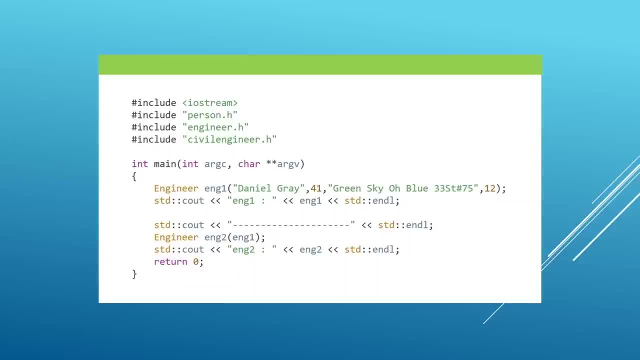 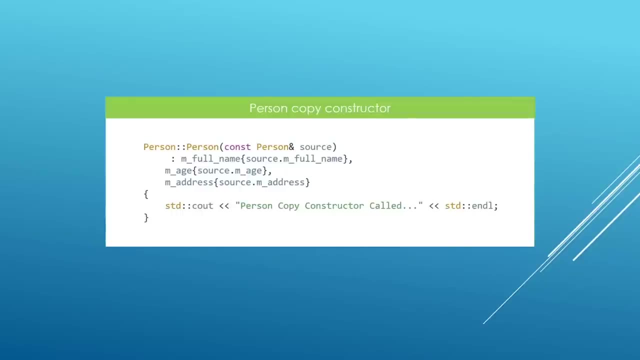 But if you happen to need to set up your own copy constructor, we're going to see how you could do that in this, And we're going to start by the base class. We're going to set up a copy constructor for the person class and this is nothing complicated. 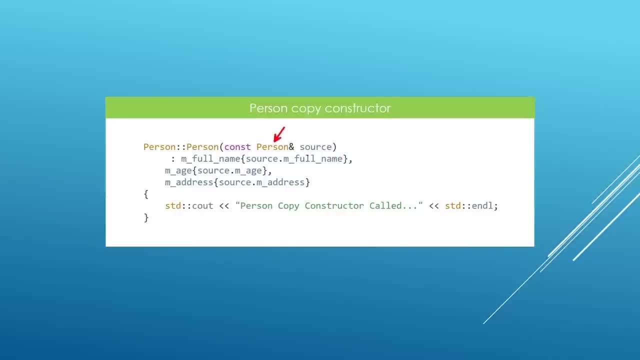 We just pass our parameter by reference. This is going to be our source object and we will be copying the data from our source object to initialize the member variables in the current object that we are copying here. Again, this is a copy constructor, which will be copy constructing from the parameter that we pass by reference. 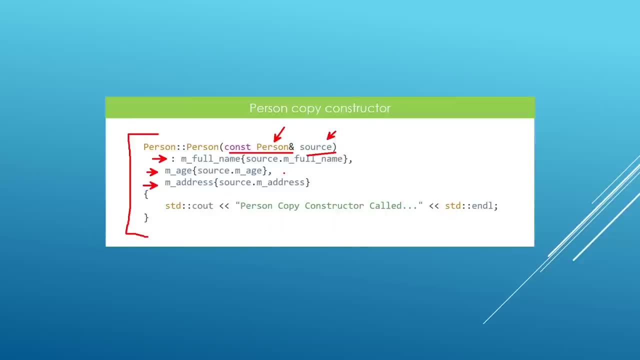 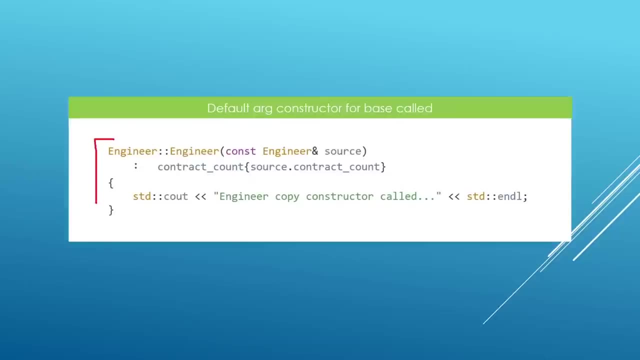 Now, how do we do the construction, The constructor for the engineer class, which happens to be inheriting from person? Try to think about that. One way to do things is to set up things like this, and this will be just initializing the engineer layer of our class, but nothing is going to be initializing the person part of us. 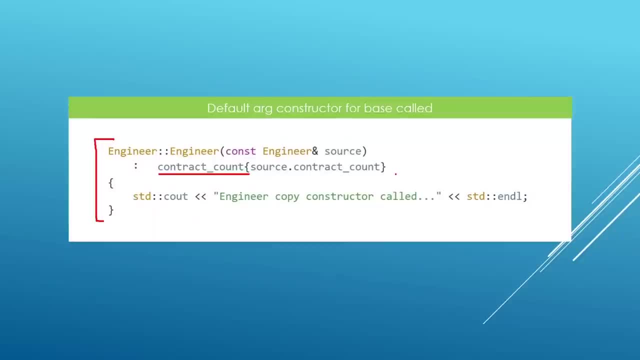 And this is bad. This is going to call the default constructor to initialize the person part of us and we will just be left in with junk data. That is Initializing the person object by default and all the data we have in our parameter engineer object is just going to be lost for the person part of us. 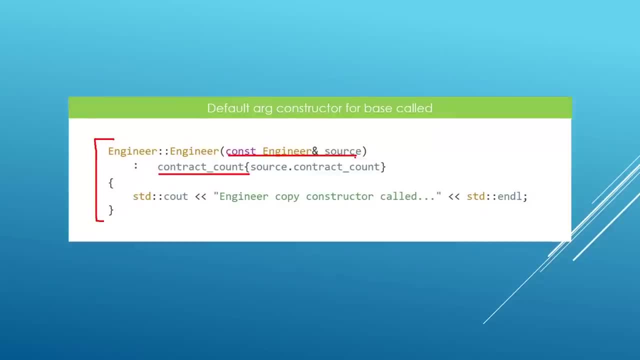 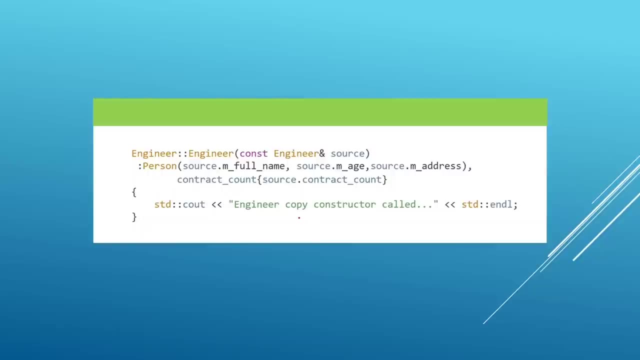 So we don't want to do this. This is bad design, You shouldn't do this. Some of you are going to say: but what if we call the base constructor? We have seen that we could do that right, But remember, this is a copy. constructor. 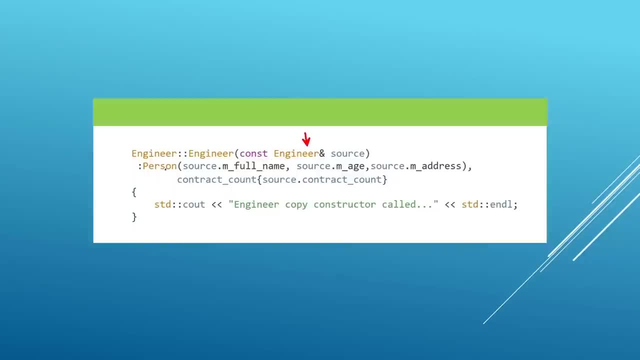 What we have on the left is an object and it happens to be that If we set up a syntax like this with the copy constructor, the compiler is going to set up a temporary person object and a copy from that object to initialize the person part of us. 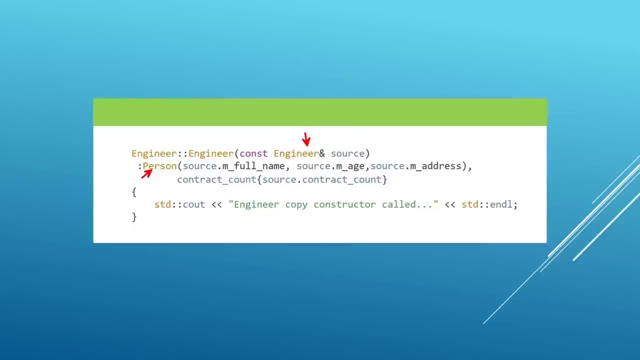 So this is going to be creating a temporary copy object containing the same data we have in our engineer object. So to some extent this is going to work. but the problem we still have is that we are using the M address member variable directly from an engineer object. 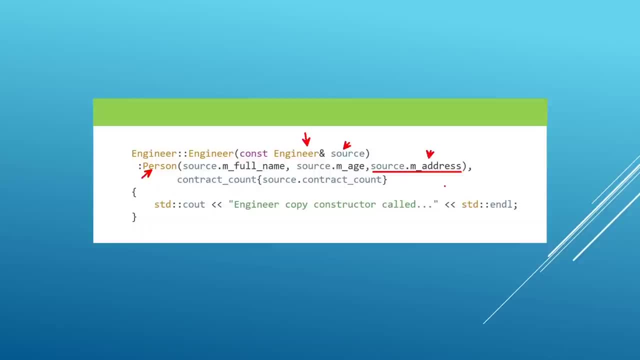 And, from what we already know, this M address member variable is private to the person class and we have no business accessing this from an engineer construct. So this is going to give us a compiler error. But you know that it is possible to set up a getter in the engineer class that is going to return this address. 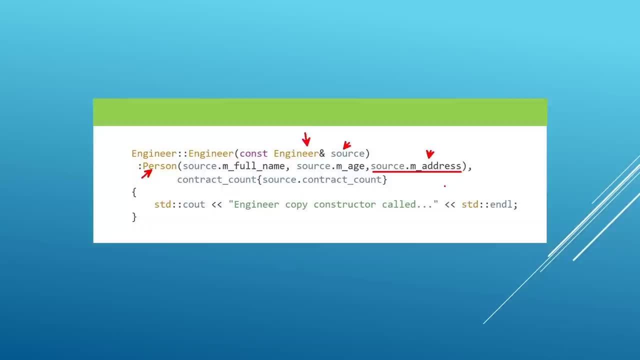 And you can call that: getter here and get this thing to initialize your data. This is going to work, but this is really weird. You shouldn't do this. This is bad design. There is a better way. I am going to show you. 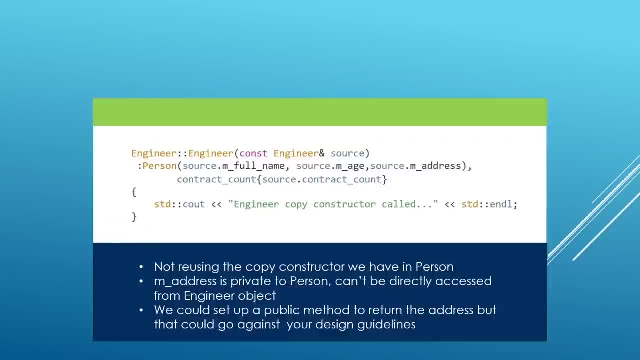 But before we look at that way, let's try and summarize the problems we have with this way of doing things. This is not going to be reusing the copy constructor We have worked hard to set up in person, So this is just going to be code duplication. 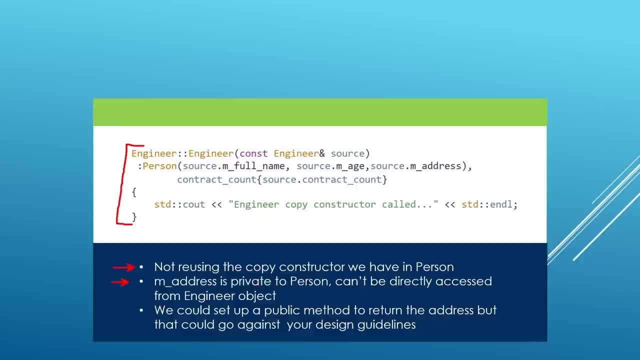 Another thing is that the M address member variable is private to person, So if we try and use it like this, we're going to get a compiler error Again. it is possible to set up a getter That Could return that And we could use that getter in this place. 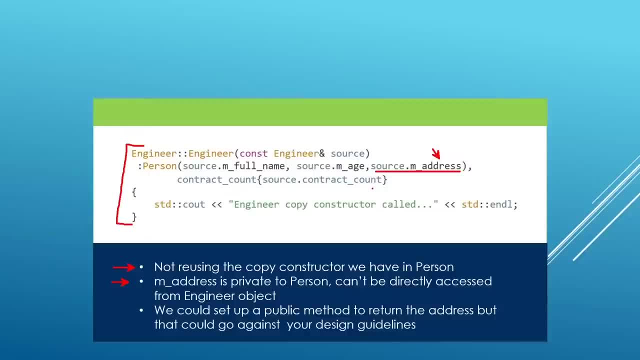 But this is bad design. We are really forced to set up a getter that is possibly only used in this place. That's bad design. We don't want to do something like this. Another thing is that this is going to create a temporary copy of person, from which we will be copying to initialize the person. part of us. 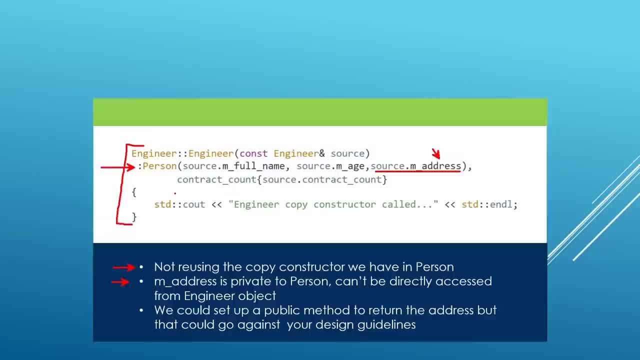 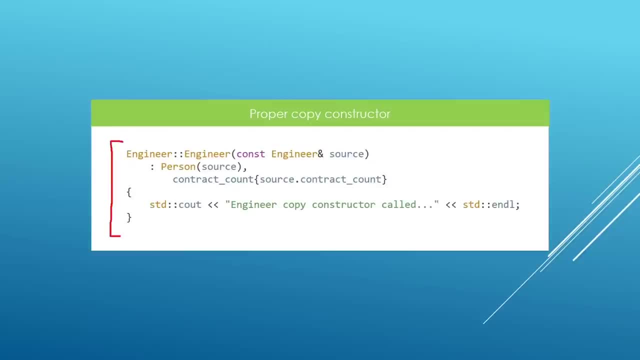 We don't want to be making that copy because we hate copies in C++ code. So the best way To do this is to set up your copy constructor in this way. We are going to say person and directly passing our engineer object. The compiler is smart enough to see that we are passing an engineer object to initialize a person object. 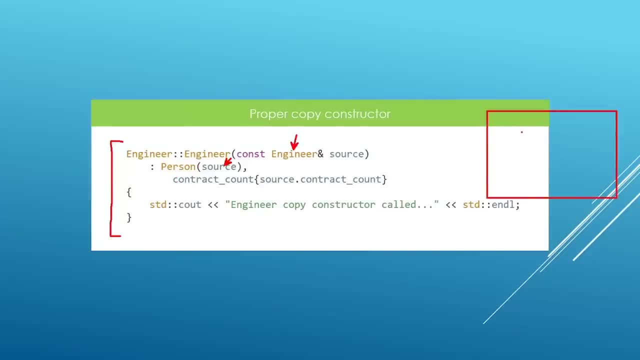 And what the compiler is going to do is really smart. Suppose our engineer object is made up of two layers. The inner layer is going to be containing the information about the person part of us And the outer layer is going to be containing the engineer part of us. 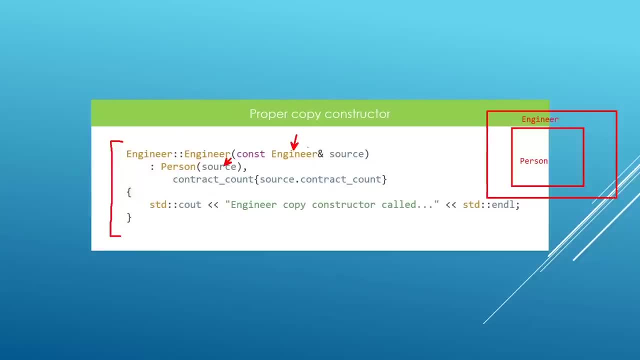 Okay, so this is the setup we have. So the compiler is going to see that we are passing in an engineer object to initialize a person object And what it is going to do is really smart: It is going to strip off all this engineer part. 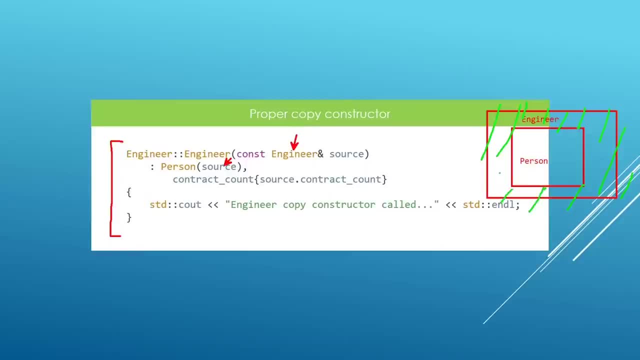 If I can describe it like this, we're going to strip off all this engineer parts that we have in our engineer object and we will be just left with the person part. If I can describe it like this, we're going to strip off all this engineer parts that we have in our engineer object and we will be just left with the person part. 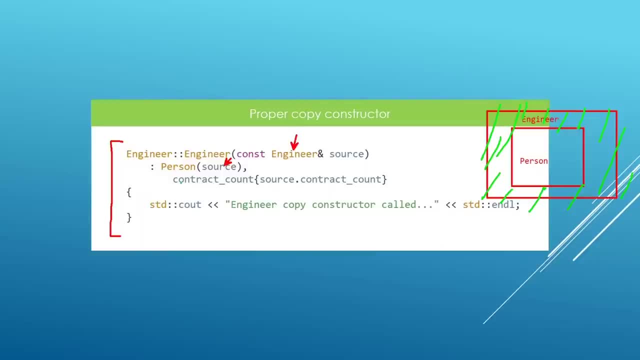 That we pass them to initialize our person object, and this is really smart and it is going to work. So again, the syntax is what you see here: We say person, we pass in our source object and then we can initialize the member variable that belong to the engineer part of us. 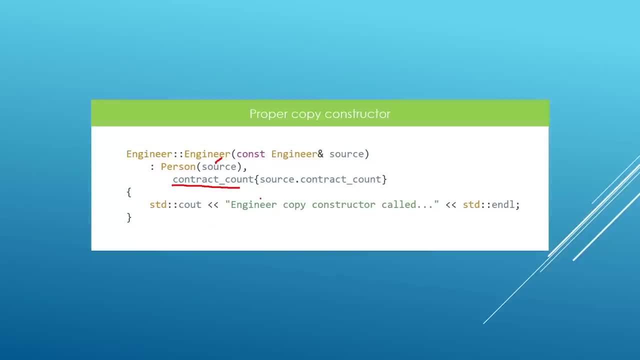 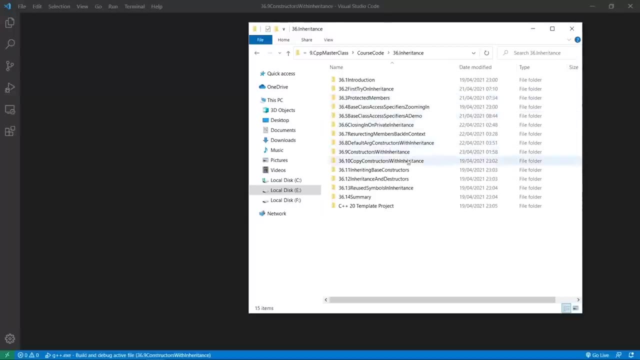 We will be initialized in contract count and this is going to work. Now that you know this, we're going to head over to Visual Studio Code and play with us a little more. Here we are in our working folder. The current project is copy. 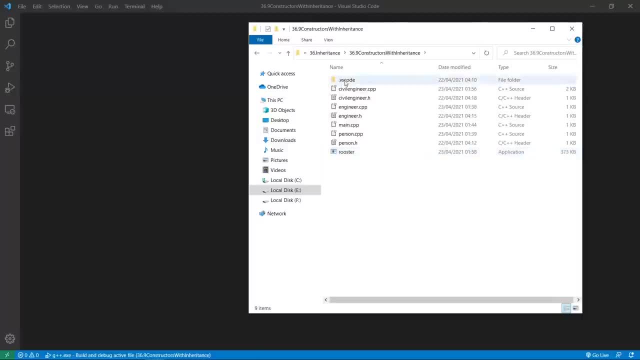 Constructors with inheritance. We will be reusing the code from the last lecture, So we're going to grab everything from that except for the binary, and we're going to copy that and put that in our current project. Let's do this And we are going to open this bad boy in Visual Studio Code by dragging and dropping here and we will have our starting point. 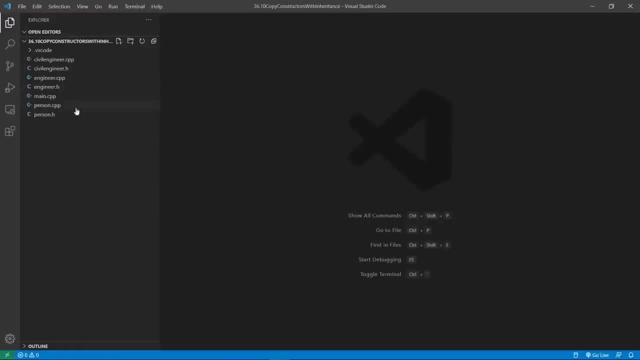 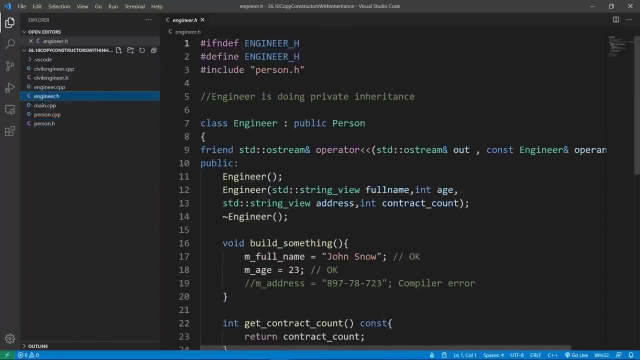 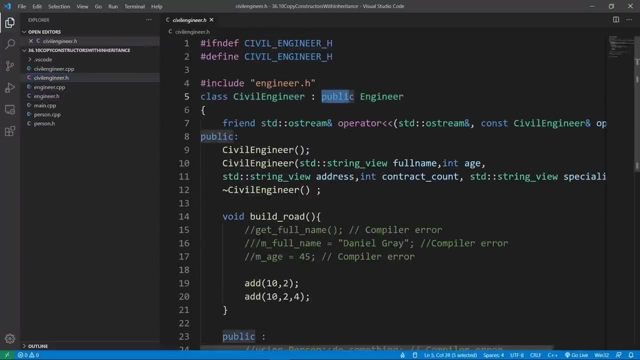 We will have our person class, the engineer class and the civil engineer class, And We Will Just be doing with public inheritance to make things easier here. So engineer is going to publicly inherit from person and civil engineer is going to publicly inherit from engineer. 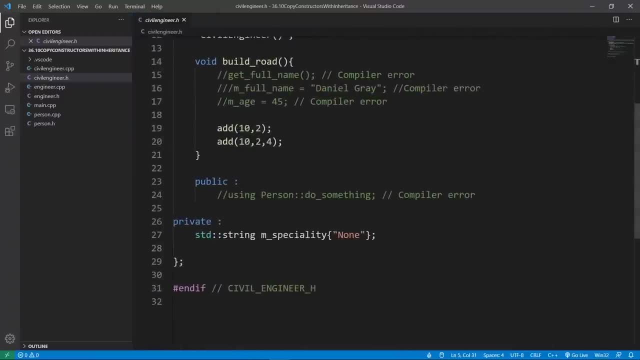 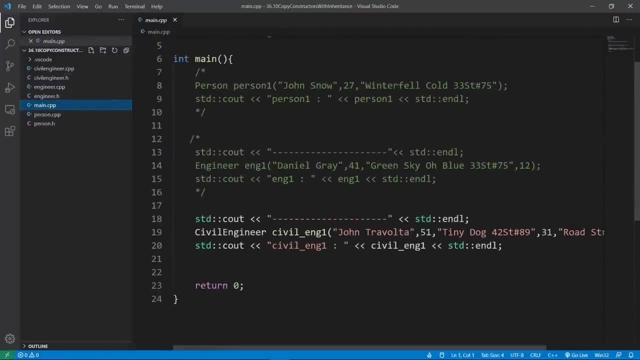 And this is everything we had from the last lecture. Nothing special. But what we want is to set up a copy constructors in such a way that we will be able to build objects from others, For example, if we leave in our engineer object. I think this is what we used in. 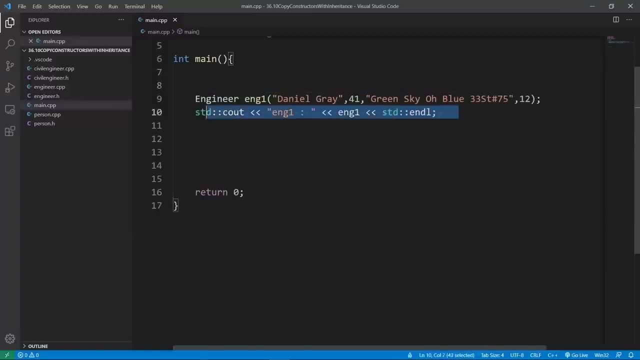 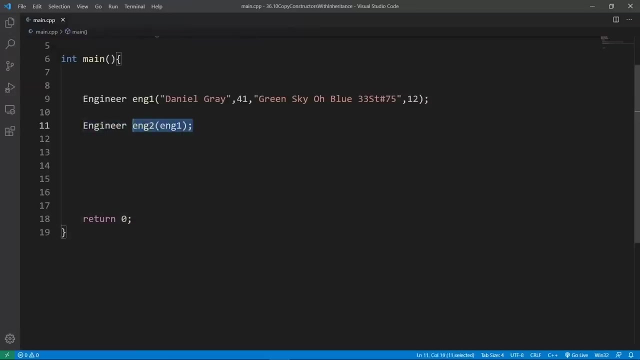 The slides. we're going to have our engineer one object. we want to be able to create a another engineer, let's say engineer two, and work that from engineer one. The thing that might be puzzling to some of you is that this is going to work out of the box even if we didn't really put in a copy constructor. but the thing is the compiler is going to insert a copy constructor for you, but that constructor is going to be member wise. 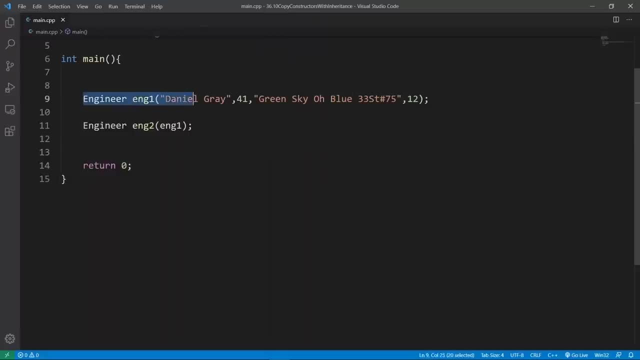 Okay, So it is basically going to be copying fence member wise. It is going to take the contract count from engineer one and copy that into engineer two And we are basically going to have the same data from engineer one in engineer two. Let's try and print: engineer two can do that. 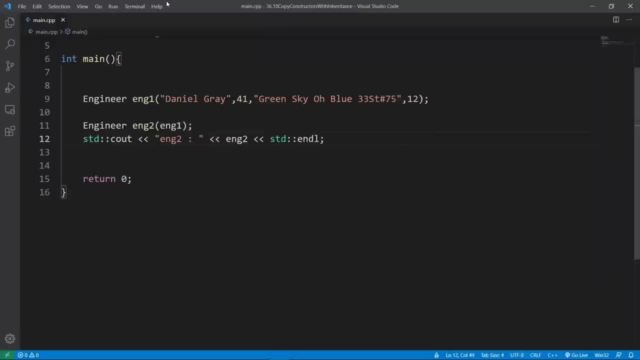 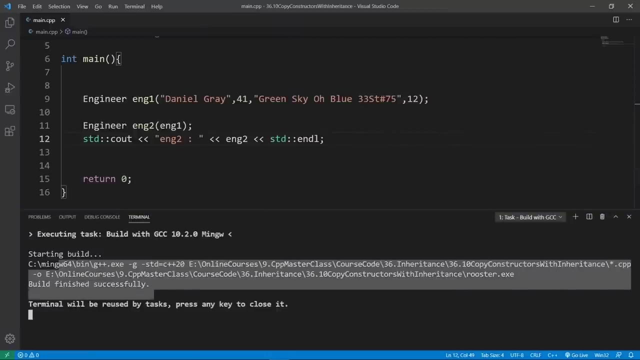 We're going to say and two, and we're going to put this out and we are going to run the task to build with GCC. That's what we want here And you're going to see that it is going to work out. 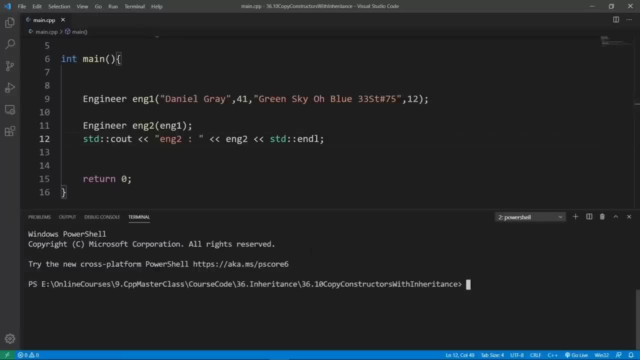 Okay Of the box. If we bring up a PowerShell window and run roaster, we're going to see that we have the data in here. We have engineer full name: Daniel gray. That's the data we have in engineer one, but notice that we are printing engineer two here. 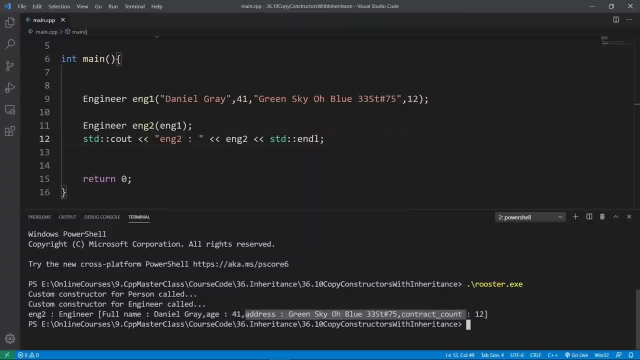 The age is going to be 41 and the address is going to be exactly what we had in engineer one And you're going to see that the constructors are going to be called to set up engineer two and the custom constructor for person is going to be called. 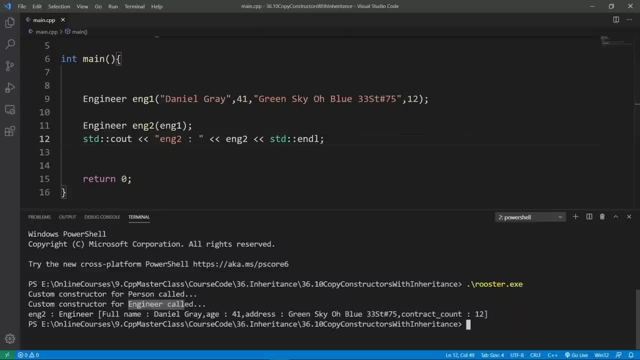 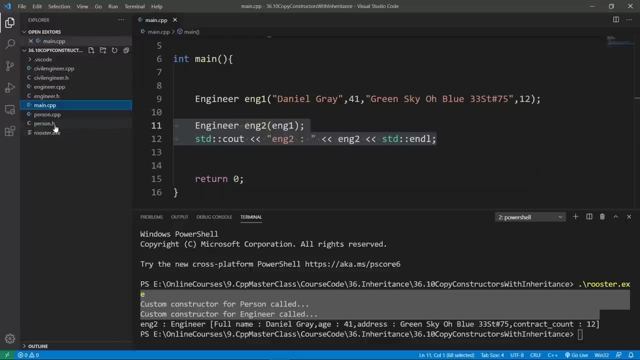 The custom constructor for engineer is going to be called, And this is exactly what we expect here. But what if we want to set up our own copy constructor and the need to do that might arise if we happen to be doing some dynamic memory allocation in our classes? suppose maybe person class has some dynamic memory allocation. 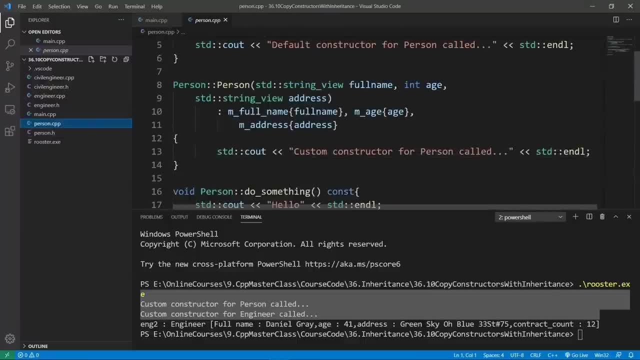 It has some pointer member variable and in the person custom constructor- we are doing some dynamic memory allocation to initialize That pointer. we may be doing the same thing at the engineer level or the civil engineer level and that will force you to set up your own copy constructor. 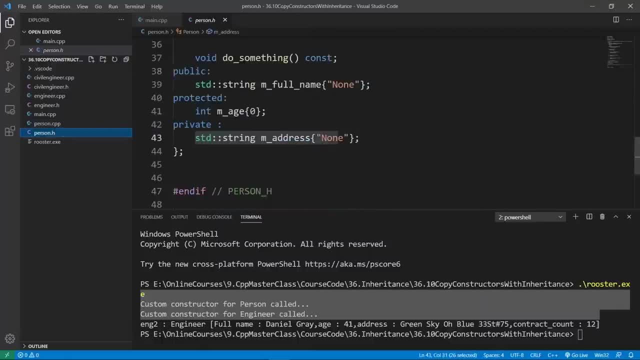 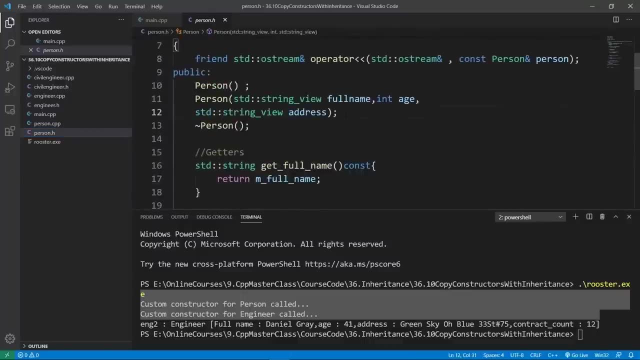 And we're going to see how you could do that in your classes. We are going to start with the person class. We're going to go on top and set up a copy constructor in front of our destructor. here We're going to say person and we're going to say cost: person, reference source. 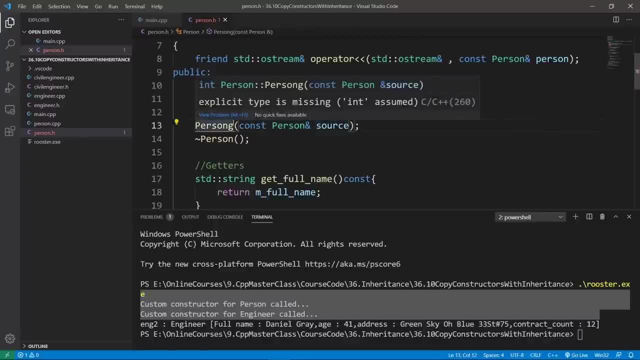 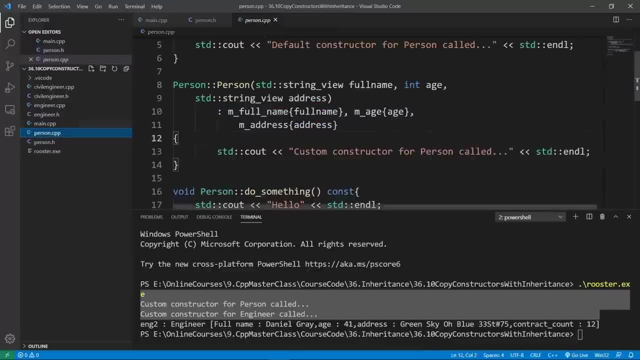 This is the syntax you use to set up your copy constructor. You already know this From a previous chapter and we're going to put in the implementation for this. We're going to go in the CPP file before the destructor, or we should go after our custom constructor. 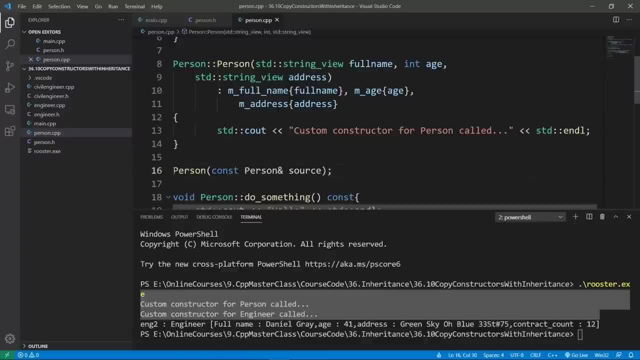 It doesn't really matter where you put this, and we're going to put in our scope resolution operator. Let's do person here, and we will just be copying data from the source person. So we're going to put in our initializer list and we're going to say m, full name. 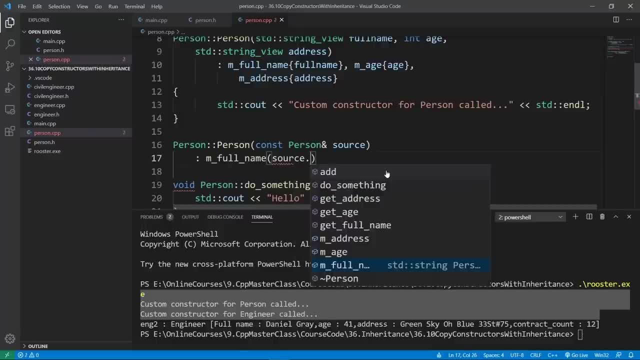 We're going to grab the name From the source person. We're going to say source m full name. We're going to initialize the age. We're going to say m age and we're going to grab the age from the source person. 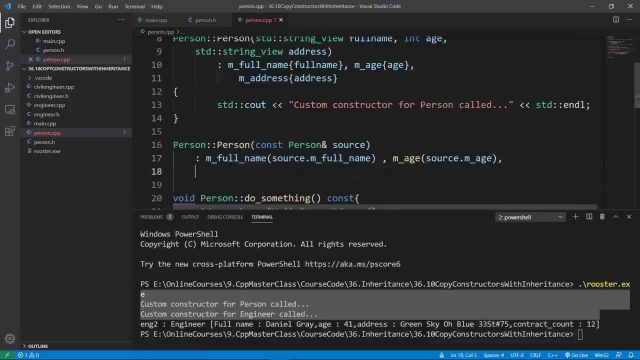 So m age here and we can go to the next line so that we see the entire thing here and say m address. And we're going to say source and say m address. This is going to set up our constructor and down below we can put in our body. 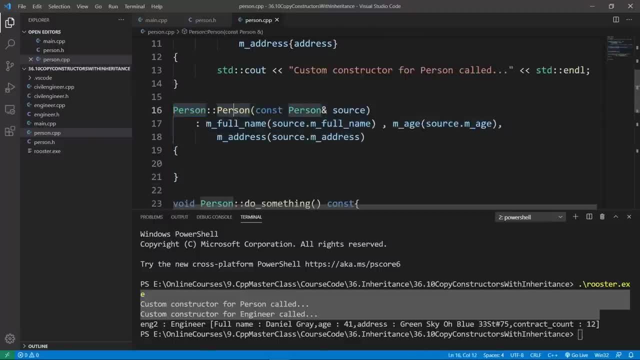 This is going to work, but this is everything we have seen so far. This is Nothing new. The syntax to set up your copy constructor: You just pass it by cost reference. If you don't pass by reference here, you're going to get an endless chain of copy constructor calls. 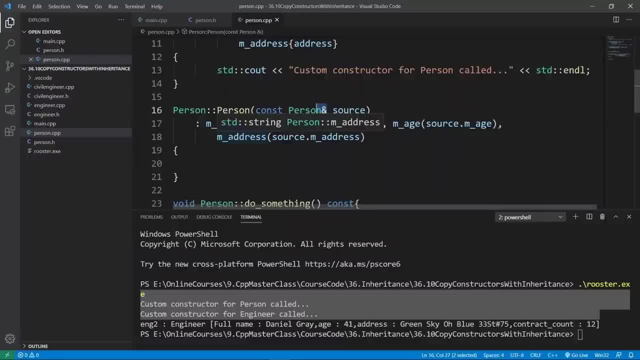 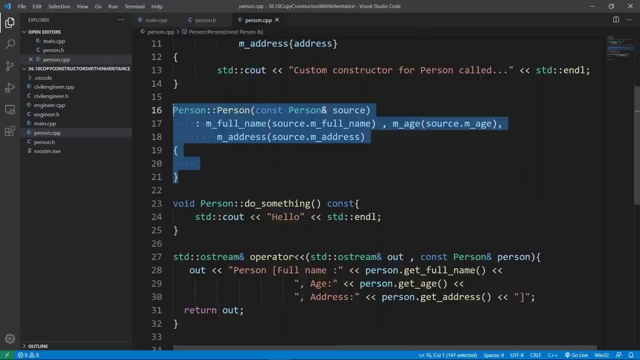 If this is confusing to you, please go back to the chapter on classes. You're going to see everything about this, and this is really all we need to do here: to have a copy constructor for a person. Now let's do things at the engineer level. 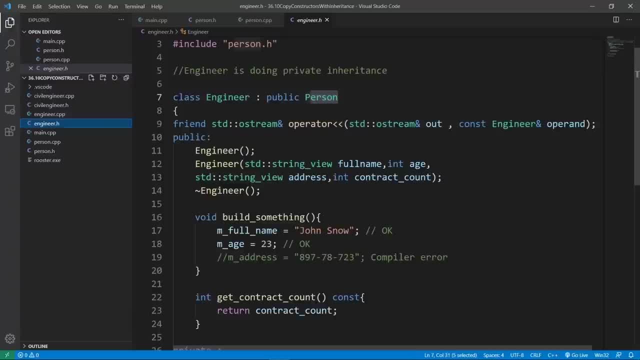 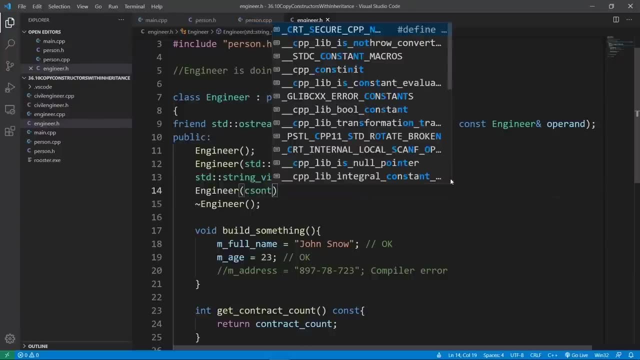 We're going to go to our engineer class and we need to set up a copy Constructor. The syntax is going to be the same. We're going to say engineer and we will be constructing from a cost engineer object We pass as a parameter here. 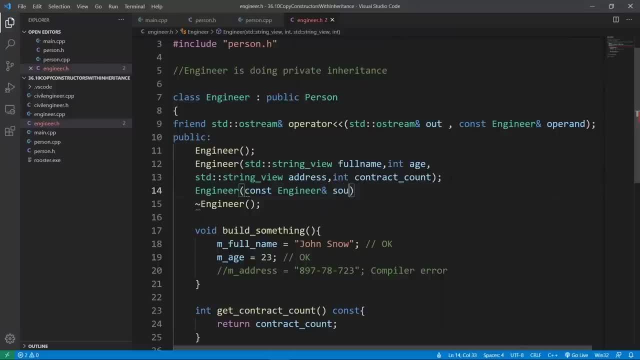 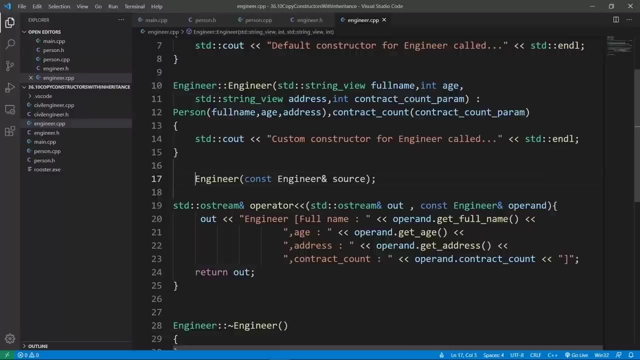 So we're going to say cost engineer by reference and say source. And the problem is going to be how we implement this thing. We're going to copy this and go in our engineer CPP file. We're going to put our copy constructor after our customer constructor and we're going to put in our scope and resolution operator. 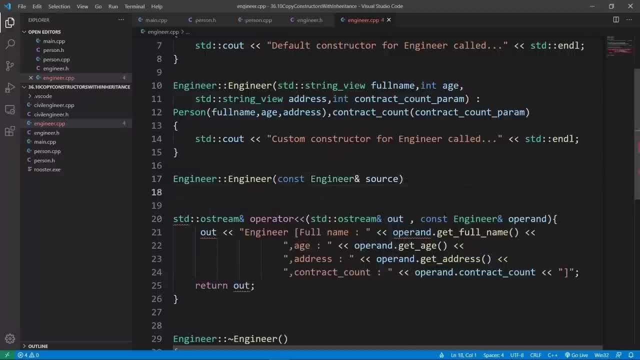 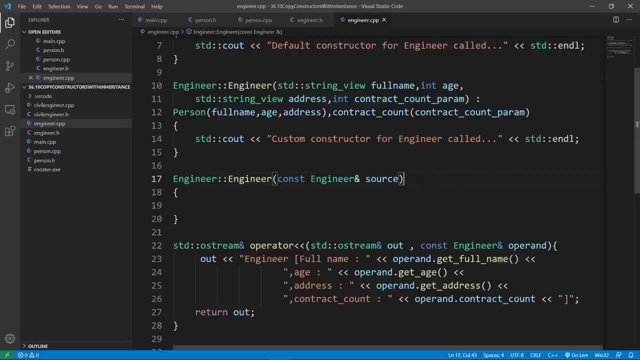 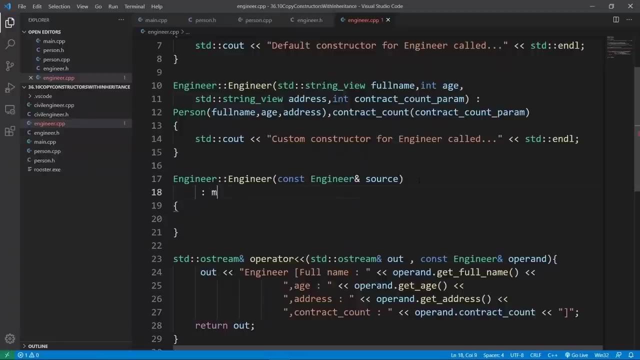 We're going to say Engineer and we're going to put in our body: Let's go below and put that if we do things like this, this is just going to initialize our engineer with junk data. We don't want that. but some of you might say, uh huh, I don't know how to call my base constructor, but at least I can initialize my contract count. 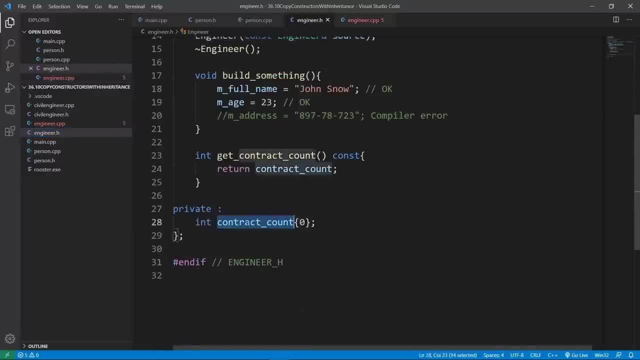 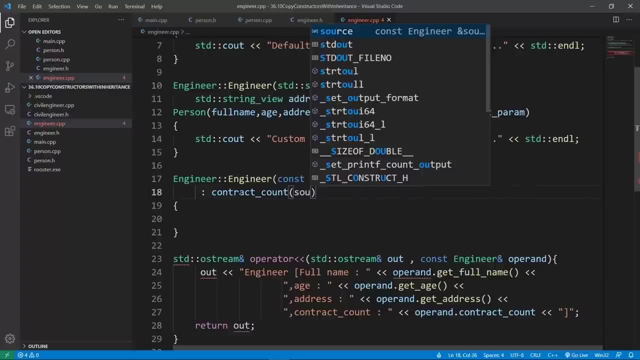 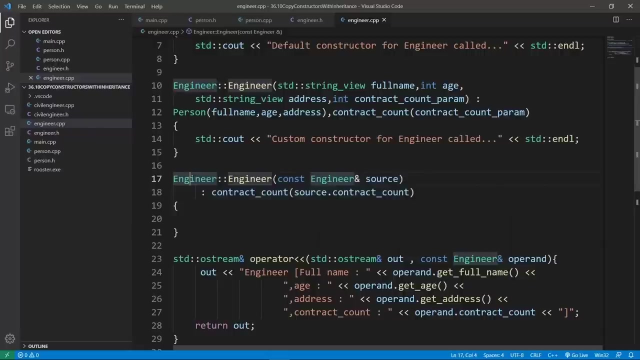 Okay, let's go back and see if we have this member variable here. Yes, it is called contract count. We can say contract count here And then we are going Okay, To initialize this with source contract count. This is going to work, but this is going to call the default constructor of person to initialize the person. part of us. 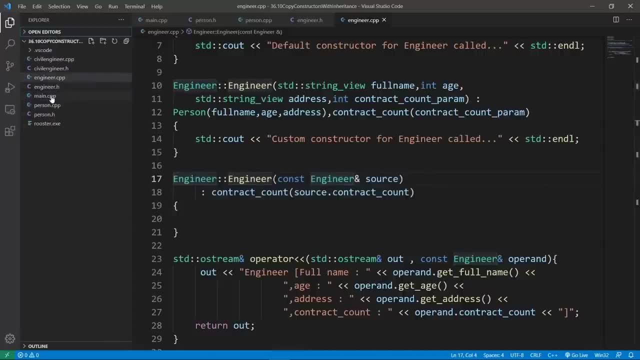 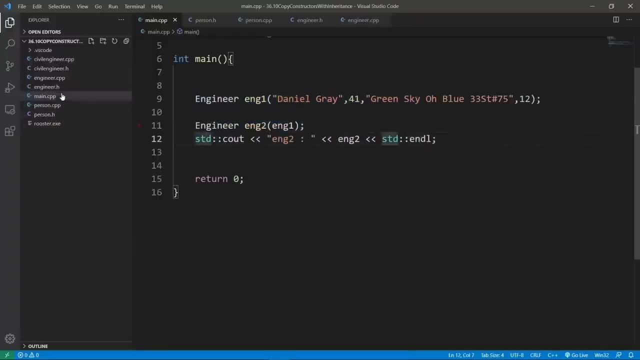 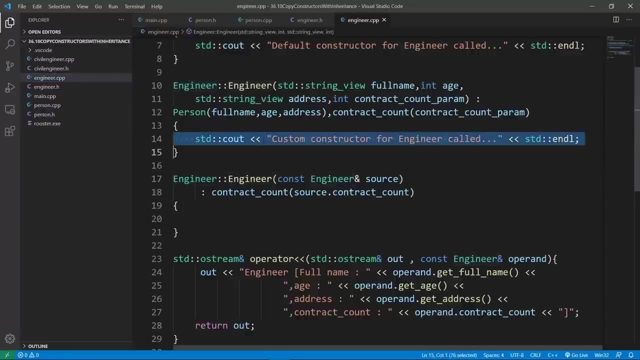 And let's go back in our main CPP file and see what we are using to try things out. We are welding an engineer object from another. Let's try this out and see if our copy constructor is called here. So we're going to say custom copy constructor called for engineer. 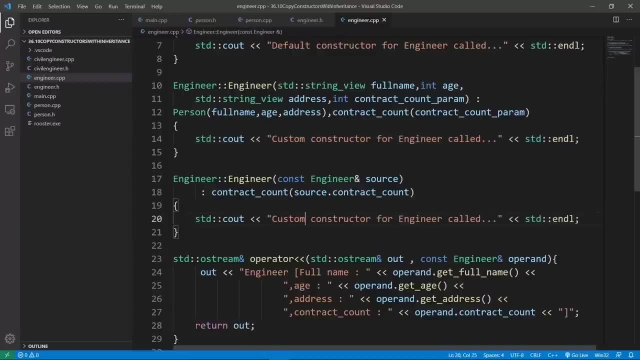 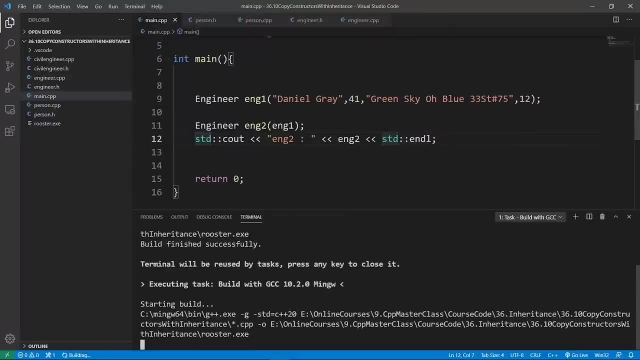 We're going to put in the message And we're going to say: custom copy constructor. And we're going to build our code: Let's weld. We're going to pass this through GCC to see what happens. The world is going to be good. 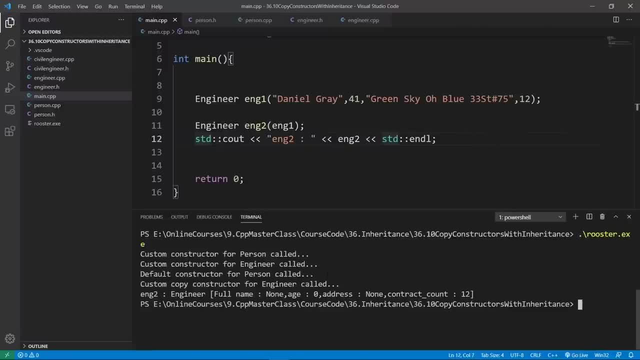 And let's see what happens. We're going to clear and run rooster. We are going to see that the constructors are going to be called to set up a person one- but we'll see that the copy constructor for engineer is called. And what I want to do to really make this super clear is put a separator between. 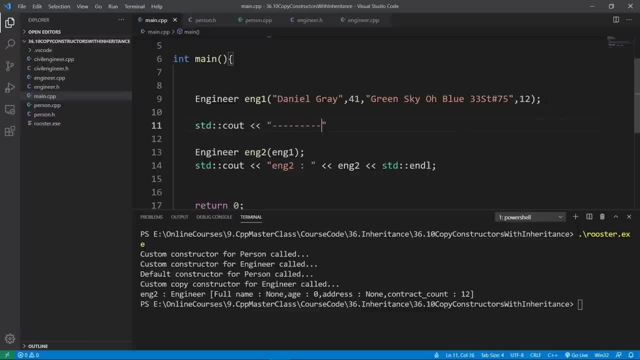 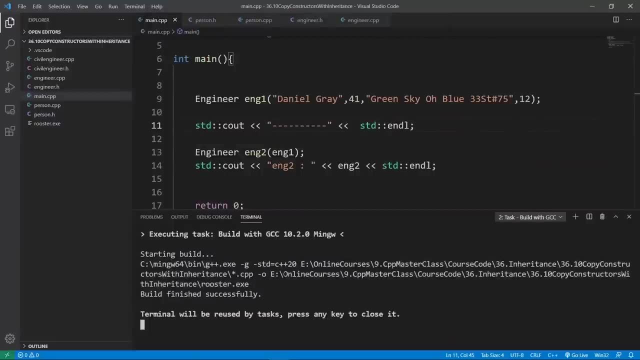 These two guys to really know what is happening here. I am going to put in a bunch of dashes, just like this. I am going to put in my new line character and I am going to build again. The world is going to be good. 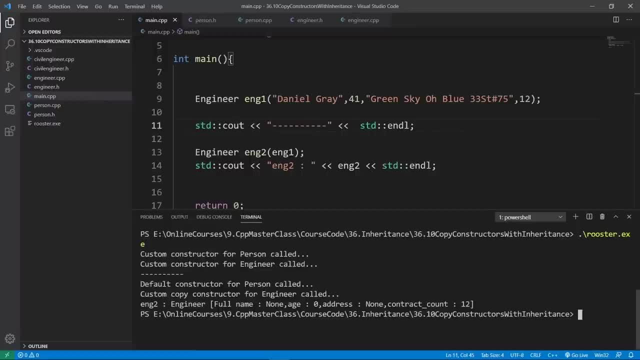 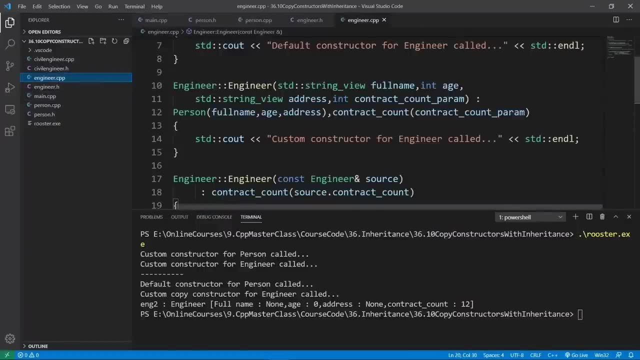 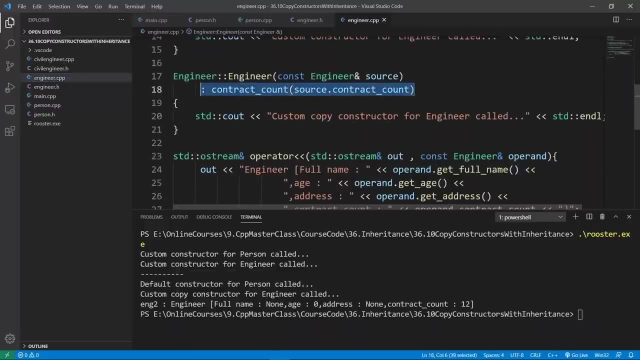 As you see, here we can clear and run rooster. Now we are going to see that the default constructor for person was called to set up the person part of us in our engineer copy constructor And the reason is we are not doing anything to call the custom copy constructor. 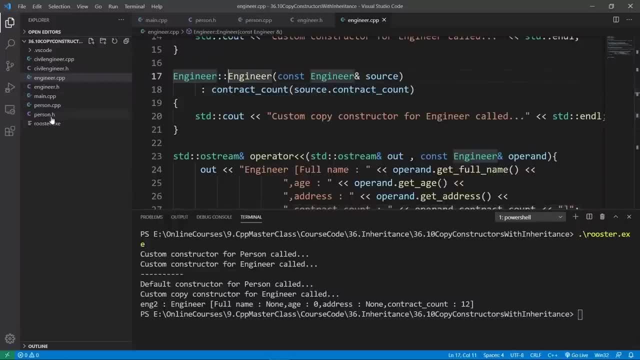 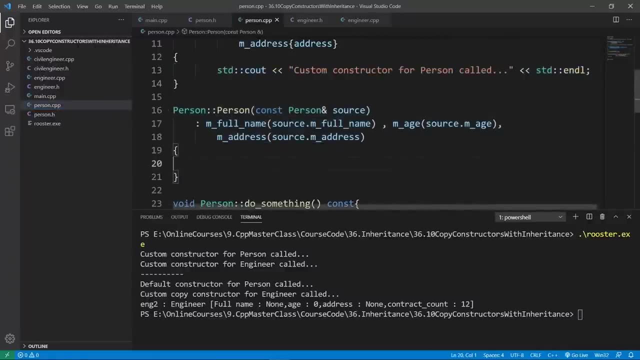 From person and let's go back in person and make sure we are printing proper information to really see this when we get to do this right. we are not putting in any message here, so we should do that. We are going to say custom constructor or custom copy constructor called for a person, but this is not called. 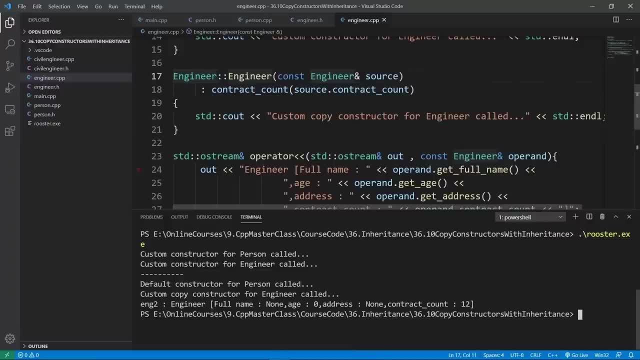 You see that we are calling the default constructor and this is going to initialize our person part with junk data. If we print engineer two here, You are going to see that the full name is none, the age is zero and the address is none. 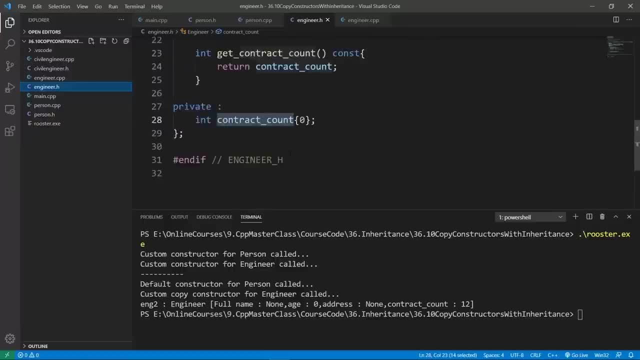 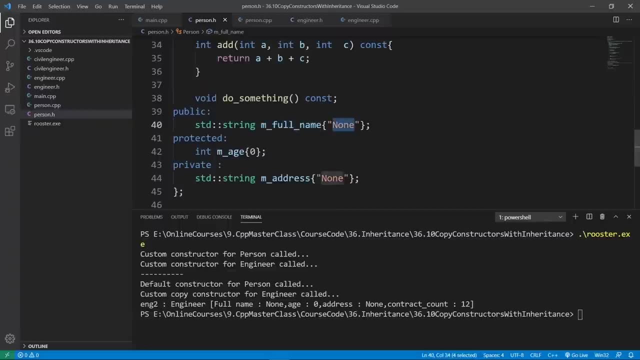 So we are basically getting the default data we have in our person objects. Let's go back and really show you that the default full name is going to be none, The default address is going to be none, The age is going to be zero by default. 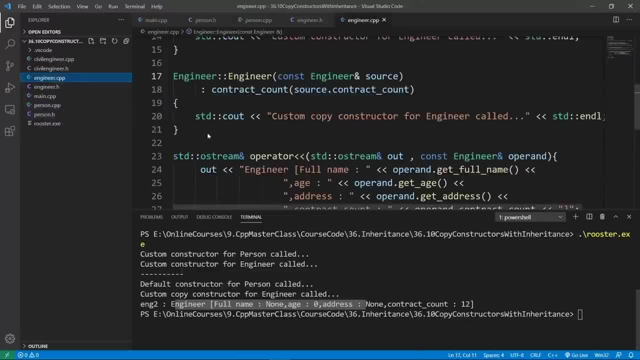 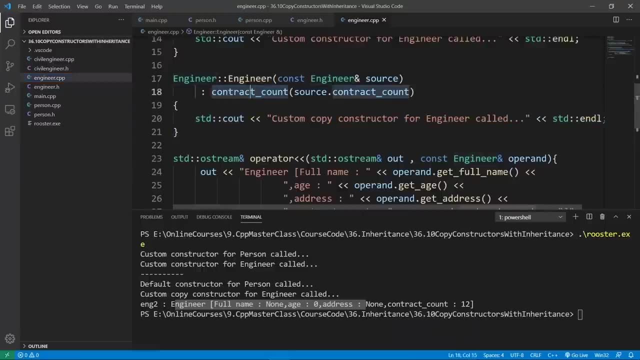 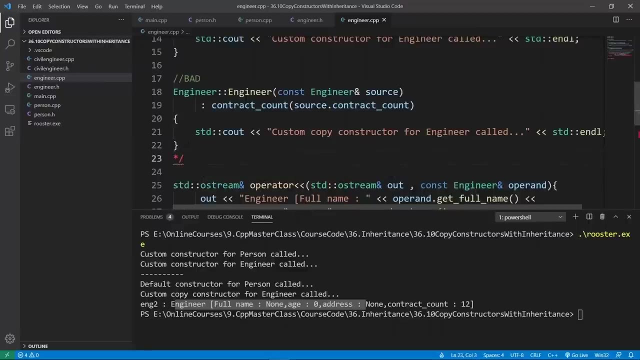 And this is what we get, because in our copy constructor we are not doing anything to get our custom constructor in person to be called Okay. So this is not going to work. This is bad. We don't want to do something like this. but let's comment this out and show you another way. 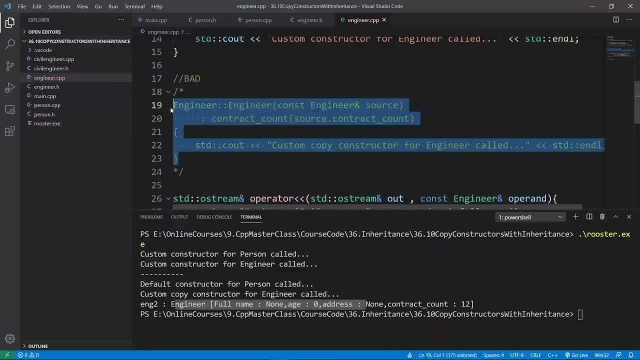 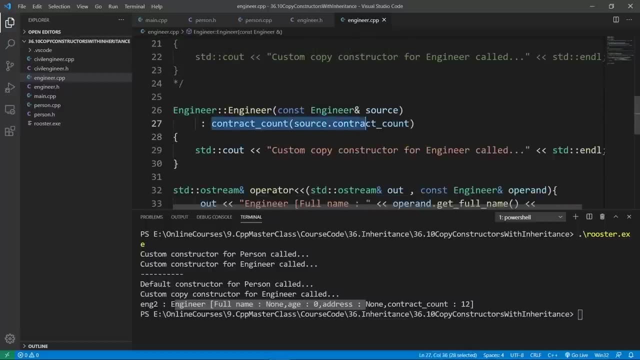 We might try to do things, and we are going to copy our copy. constructor, Let's go down and do this. We're going to put in another copy of this, but we don't want to just initialize our contract count member variable. Instead, we want to do something else. 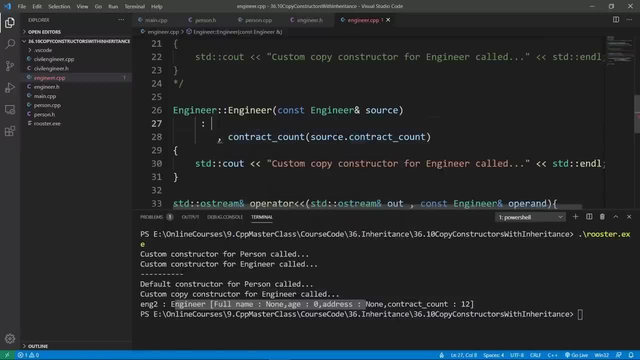 We're going to put a comma here and we're going to say person. Some of you might be thinking: what if we call the base constructor directly? We can do something like this: We can say person and we can say source and full name. 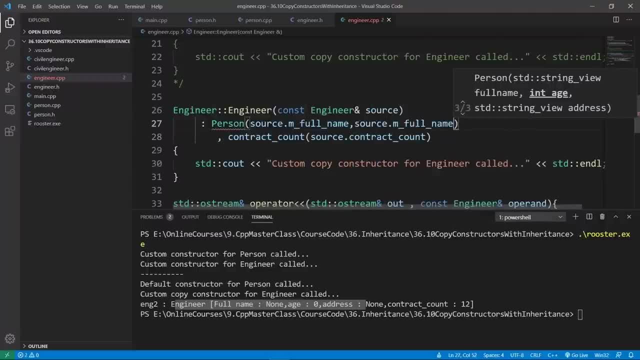 We can do that. We can say source M H and some of you are going to say source M address. Let's do that: source M address and we're going to build a person object and use that to initialize the person part of us. We are basically going to be calling the other person constructor that we have, which takes three parameters. 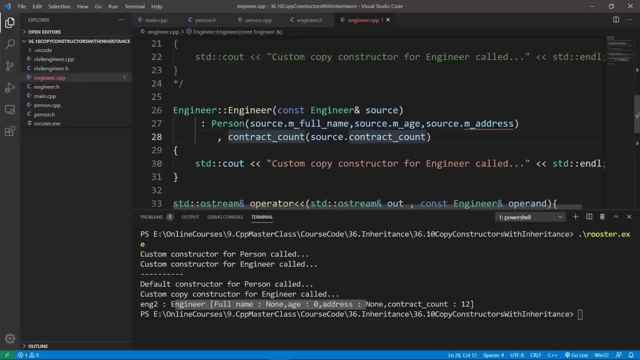 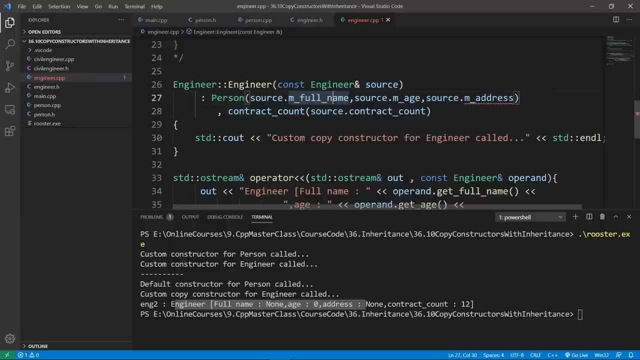 This constructor here. This is what we are trying to call in our copy constructor, But, as we saw in the slides, this is going to have a bunch of problems. This is going to be creating a temporary person object that we are going to be copying from to set up the person part of us. 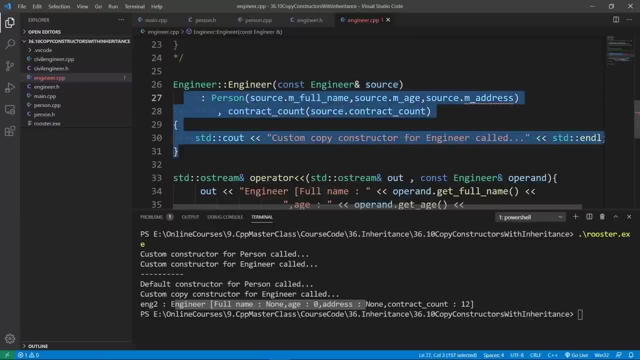 But another problem we have which is actually going to cause a compiler error is that we don't have access to the M address member variable from an engineer constructor And this is going to give us a compiler error. Let's actually try and compile this program to really show you this. 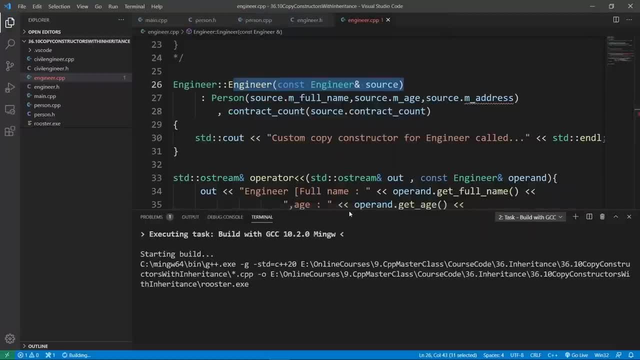 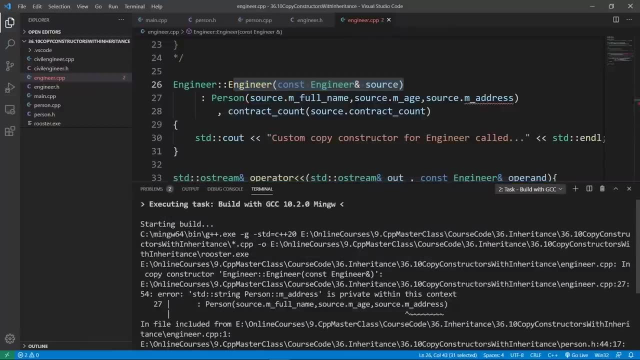 We are learning, we should really see as many compiler errors as we can. So the world is finished with errors And if we go up we're going to see that our error is the M address member variable is private to the person class And we have no business accessing that in the engineer CPP file at line 27 in our constructor here. 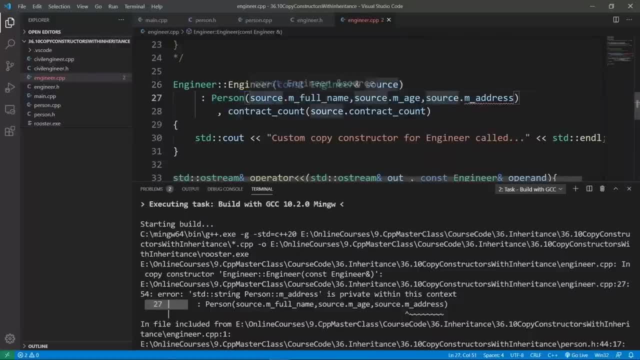 And this is going to be our offending line: We can't do this. One could go in our person class And set up a public getter method which is going to be inherited by engineer, And we could call that to return the address. 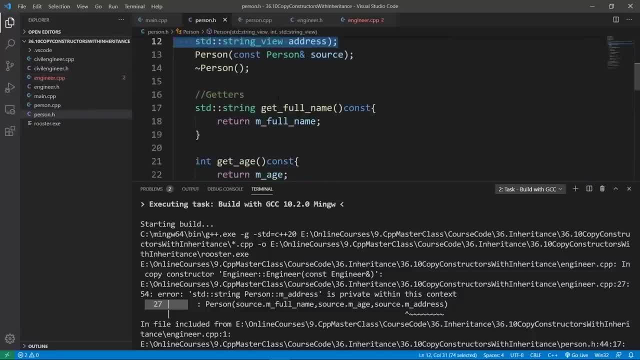 Let's actually do that to show you that you can do that. So we are going to go in and put in a public method which is going to return the address. We actually have that here, So we can call that, We can say source, get address. 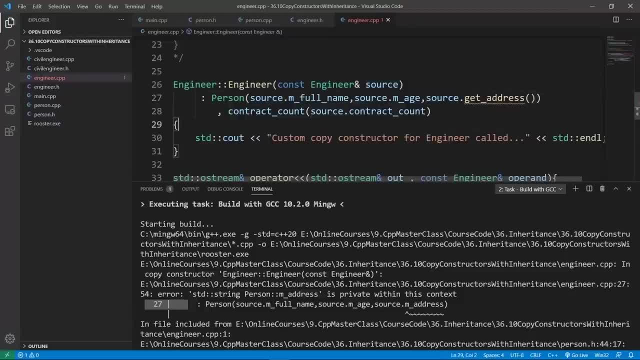 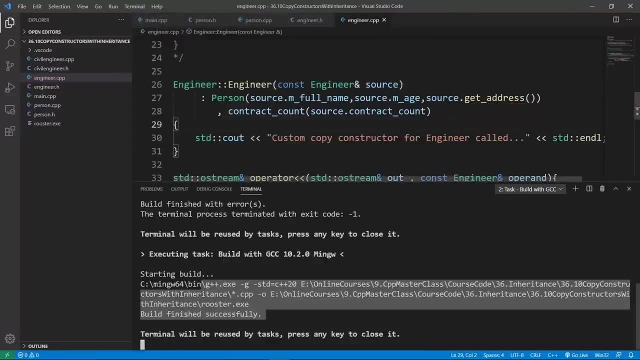 This is going to work. This is going to set up our thing. Let's try to build, because I think a Visual Studio code is missing With us here. Okay, You see, the both is good. It is Visual Studio code which wasn't understanding our code here. 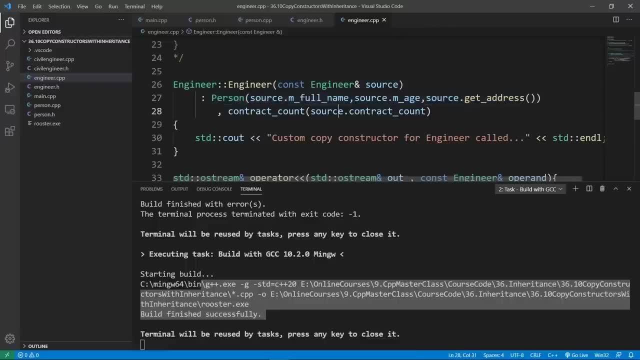 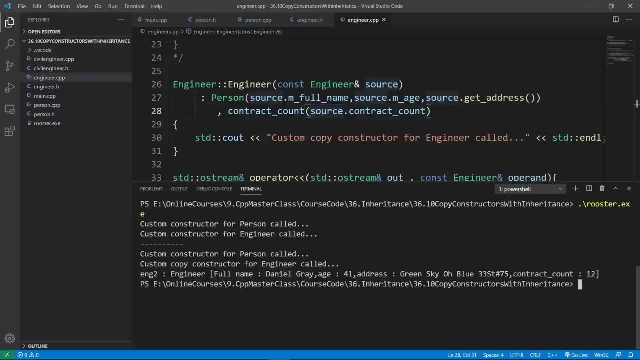 And if we run our program, we're going to see that things are going to work exactly as we expect. Let's actually run the program here. I'm going to clear and run roaster. We're going to see that now the information is being forwarded properly. 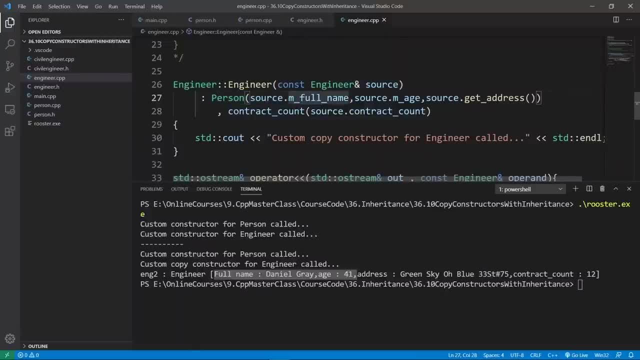 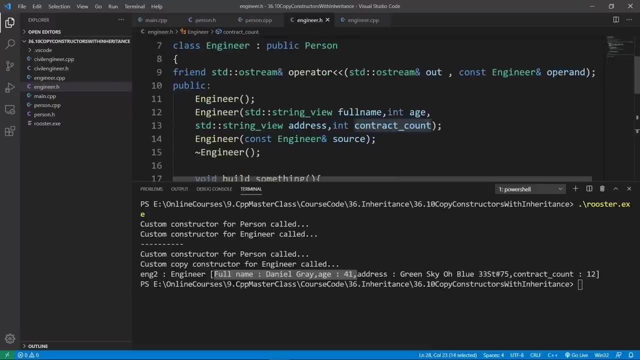 But we are setting up a temporary person copy which we are copying from to then forward the data to the person part of us. This is not good design, And what we really want is the setup that is going to allow us to call the copy constructor that we worked hard to set up in our base class. 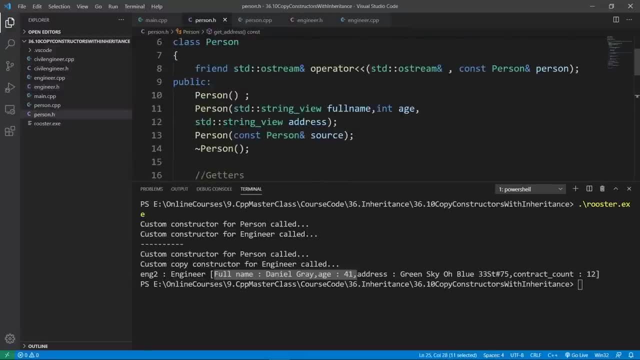 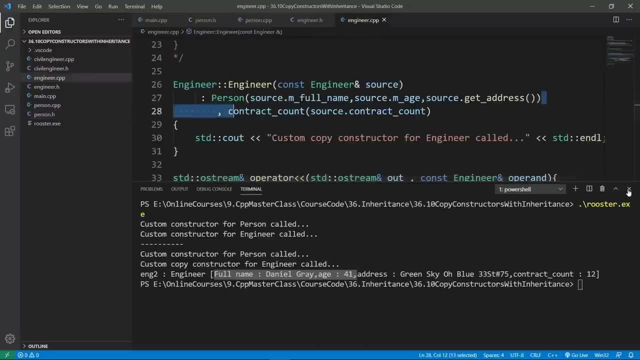 Let's go back to person and see that if we go up, we're going to see that we have a copy constructor We really worked hard to set up. We want to reuse this in our engineer class And that's what we're going to see here. 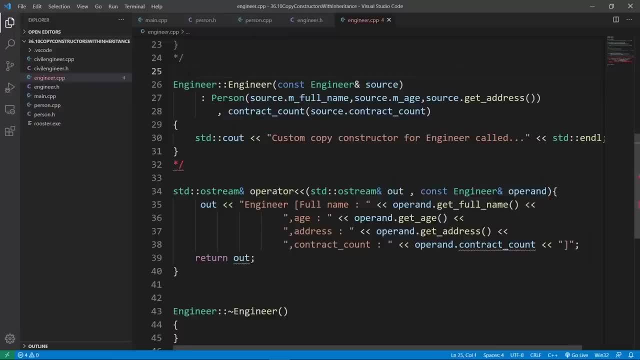 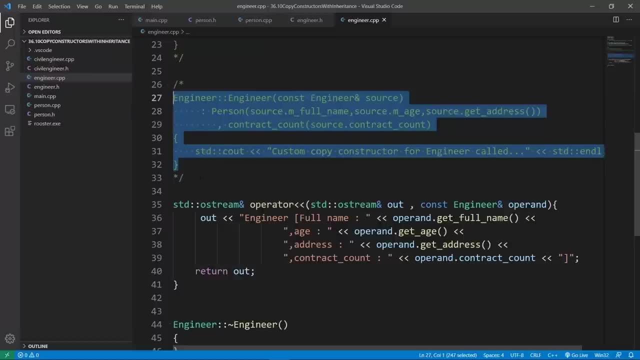 So this is working, but it is not optimal And we should read it. Let's try to reuse our code as much as we can. So what we're going to do is set up a mechanism that is going to reuse the copy constructor we have in person. 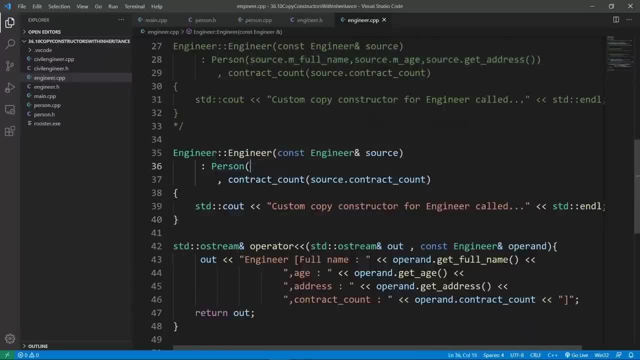 And all we need to do to get that to work. we can say person and then call the copy constructor of person by directly passing in our source object. Notice that we don't need to set up a temporary person object. We will directly be copying from our engineer object. 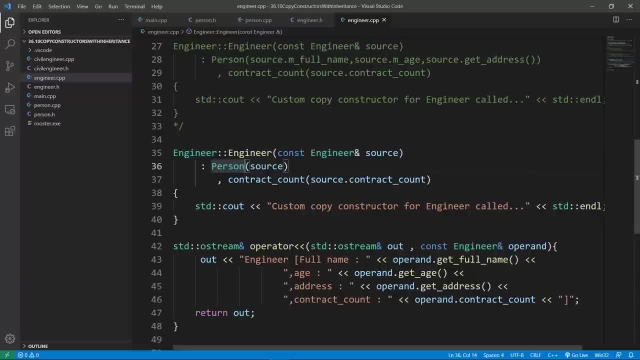 But this is going to do this, So we're going to do the slicing we saw in the slides. Again, if we have two layers on our object, the inner layer is going to be the person part of us And the outer green layer is going to be the engineer part of us. 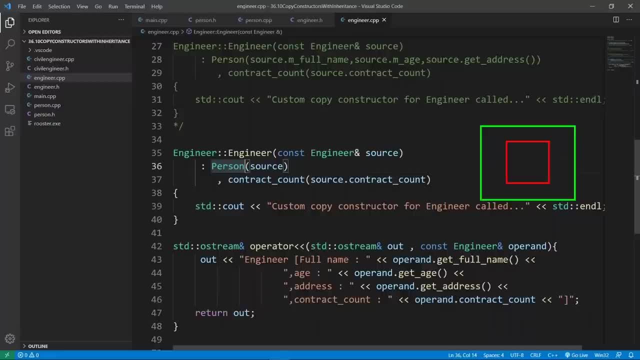 What the compiler is going to do. the compiler is going to see that we are actually passing in an engineer object to initialize the person part of us here, And it is going to see that we just need the red part. We don't need the green part. 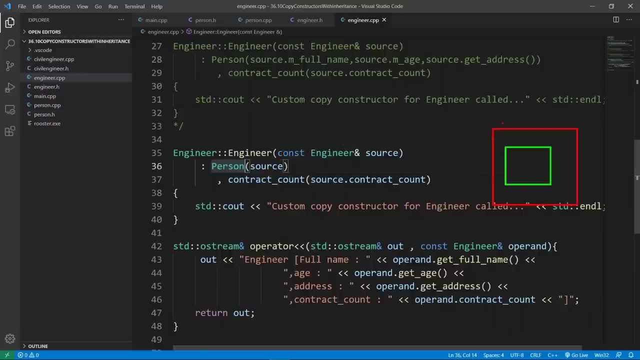 The green part. here The compiler is really smart, so it is going to slice off the outer engineer layer and only leave in the green person part And it is going to use that to initialize the person part of our engineer object. And this will be reusing the copy constructor we have in our person object. 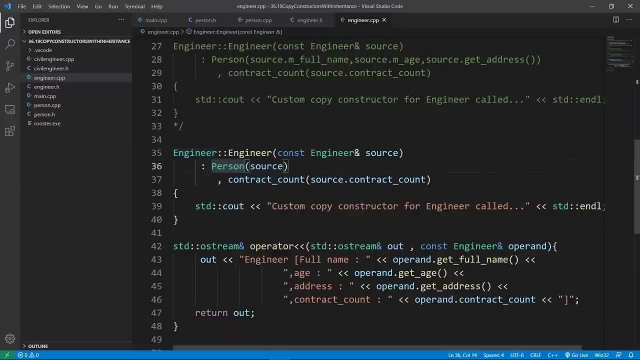 And this is really cool. This is the optimal way to set up your copy constructors If you have an inheritance, So let's try and build the code again. We're going to pass this through GCC to see if this actually works. The build is going to be good. 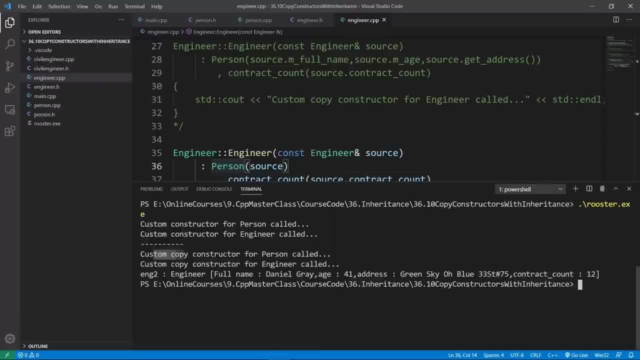 We can clear and run rooster. We're going to see that the copy constructor is going to be called for a person to set up the person part of us And then the custom copy constructor for engineer is going to be called to set up the engineer part of us. 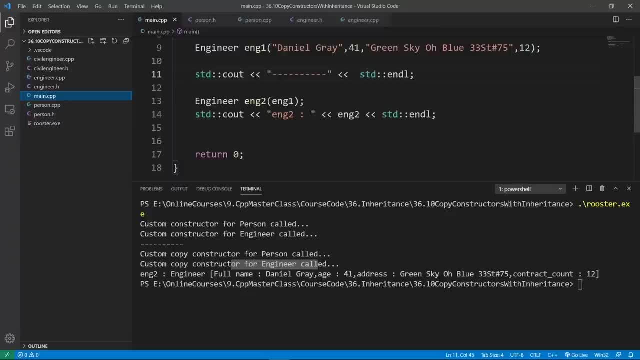 And if we look at the information we have in the main function, we're going to see that it is the same data. Then you gray for the full name. Age is 41. Address- is this gibberish here? and the contract count is 12.. 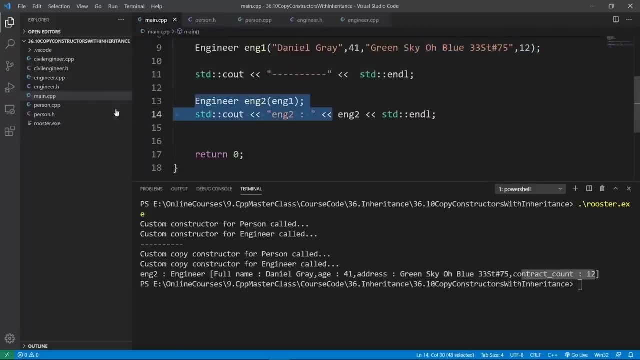 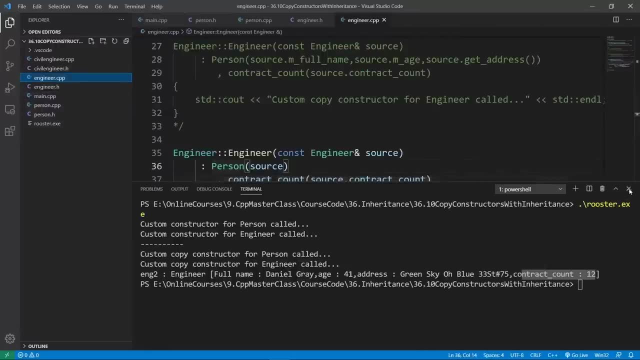 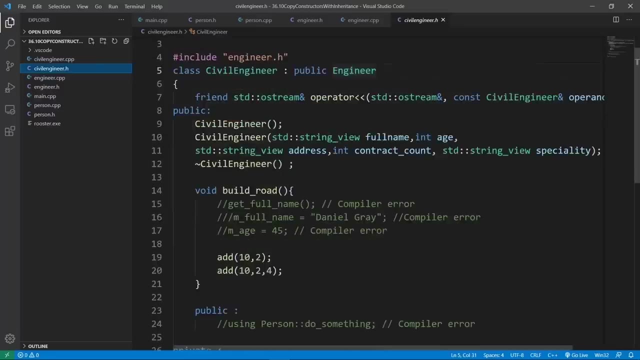 It is exactly what we passed here And our copy constructor is working. Now that we have this working, we can safely reuse the same ideas in our civil engineer copy constructor. We can head over in our civil engineer and set up a copy constructor. 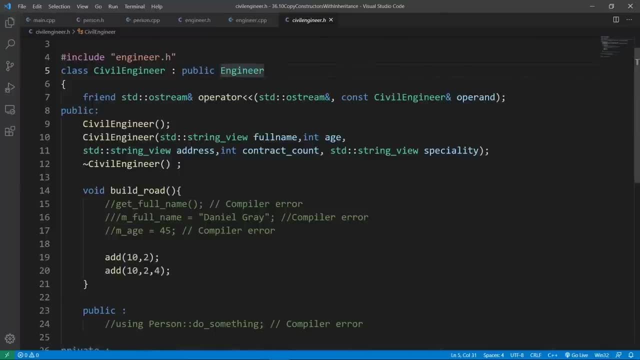 So let's do that. We can close the left side bar here so that we see the entire thing. We are going to say civil engineer and we want to set up a copy constructor. So we're going to say const civil engineer here and we will be passing this by reference. 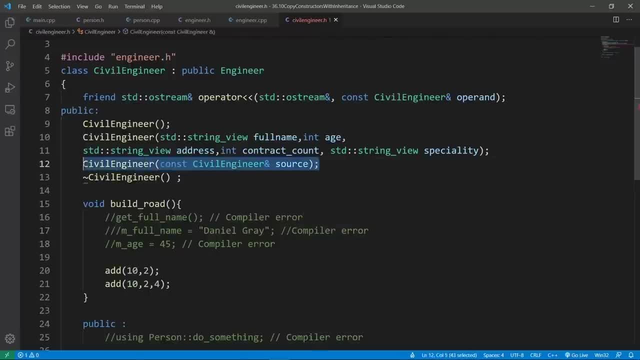 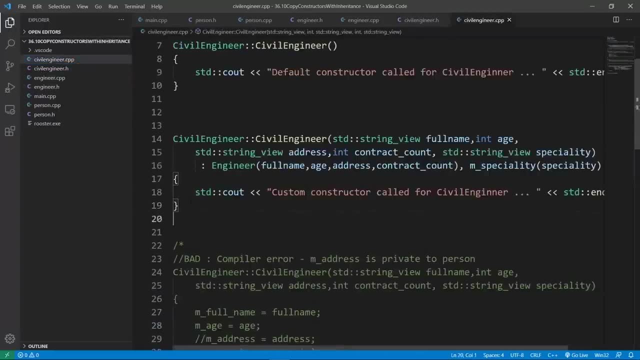 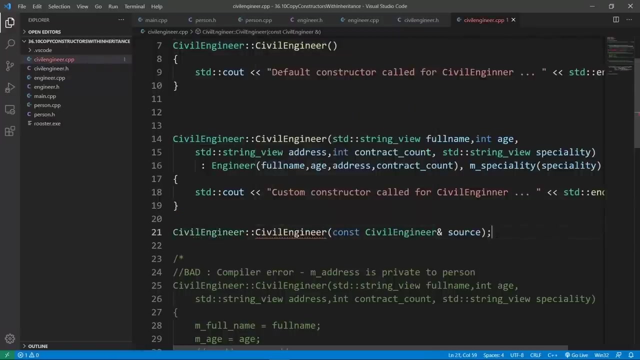 We're going to say source and we're going to put the implementation of this in our CPP file. We can hop over there and go below our custom constructor. We can put in our constructor here. We're going to say civil engineer and put in our scope resolution operator, and we're going to go. 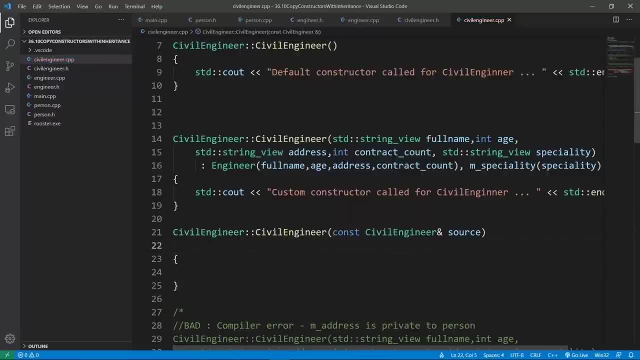 down and put in the body And in our initializer list we're going to call the copy constructor from engineer because, remember, civil engineer is inheriting from the engineer class. So we are going to call the engineer copy constructor. We're going to pass in source. 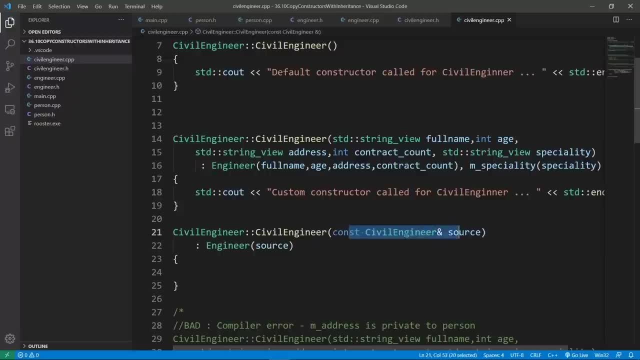 And again, this is going to slice off the civil engineer port and only use the engineer port of us to construct an engineer object from this slice stuff. Engineer Object we get from our copy constructor here And this is really cool. After that we will initialize our contract. count: member variable. 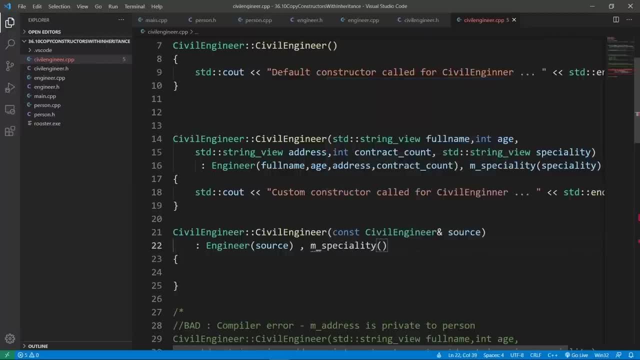 It is M speciality, if I remember correctly, And we're going to grab source M speciality and we will use that to initialize the civil engineer part of us here. Let's go in and say that the custom copy constructor is being called here and we're going to say custom copy. 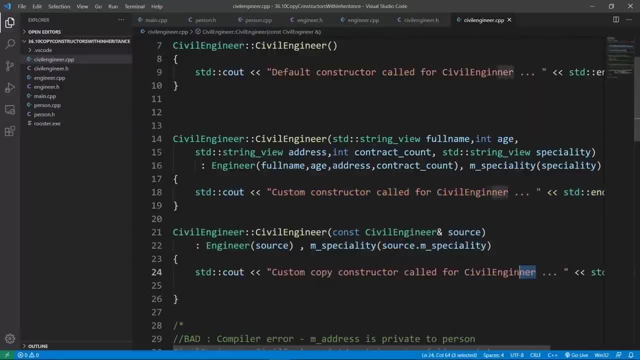 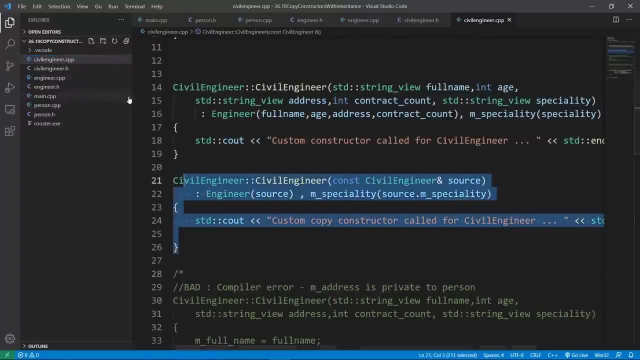 constructor called For a civil engineer. What did we do here? We said: engineer, Let's do engineer. This is what we want, And we're going to say engineer here properly. Sorry for this, but this is no big deal. And now that we have this in place, we can actually build civil engineer objects and copy constructed them. 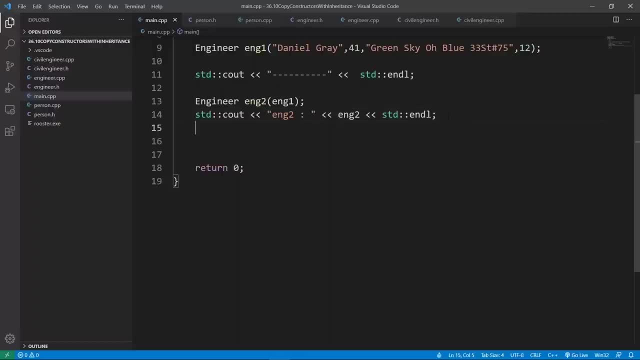 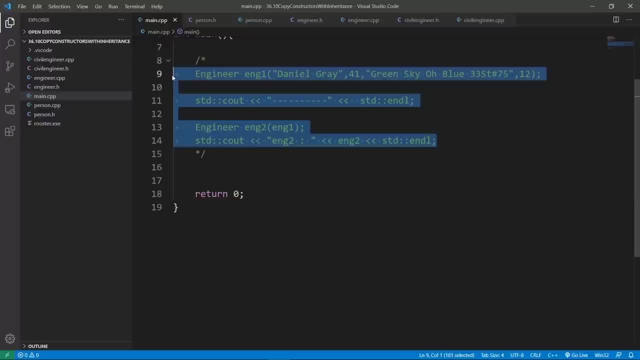 We can comment out the engineering stuff we have and we can just put this in a block comment and we're going to copy: construct civil engineer. How cool is that? We're going to set up a civil engineer. Let's do that. And this is going to be a civil engineer and we're going to say Daniel Gray. 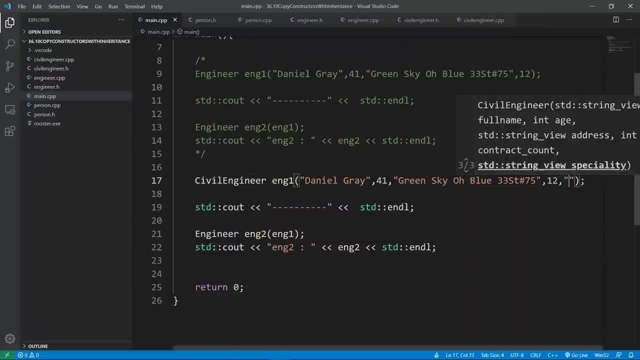 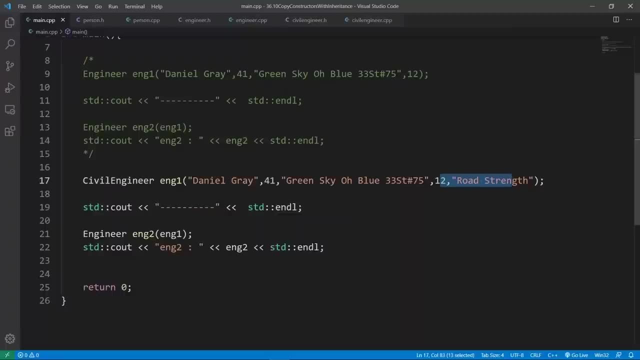 We're going to put in all the data and we're going to specify the speciality to be road strength. This is something that just made up, I don't even know if this kind of speciality exists- And we will set up another civil engineer object called and two, which we are going to be copy construction from, and we will see. 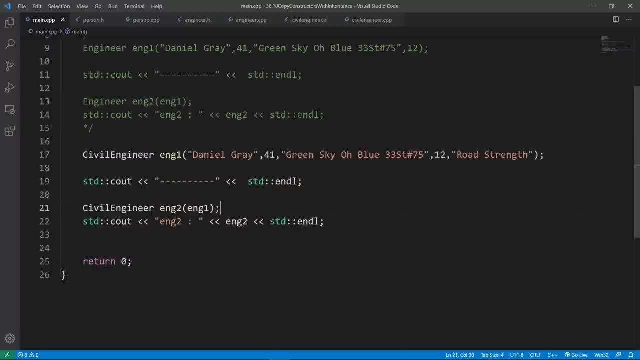 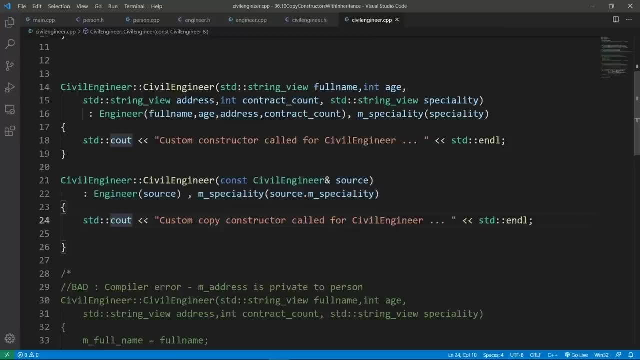 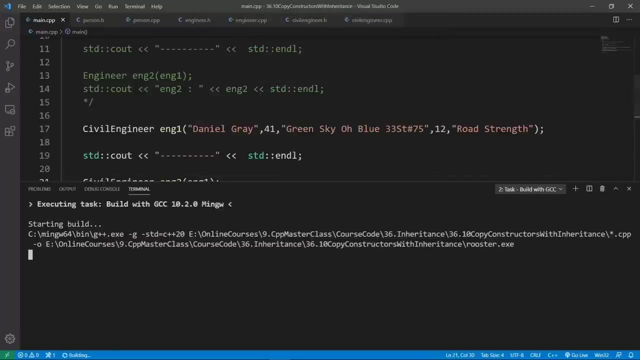 what happens when we copy construct this thing here. We should call our copy constructor in civil engineer and things should propagate up all the way to the person part of us And we're going to see what happens. Let's build this code. We're going to pass this through GCC, as we always do. 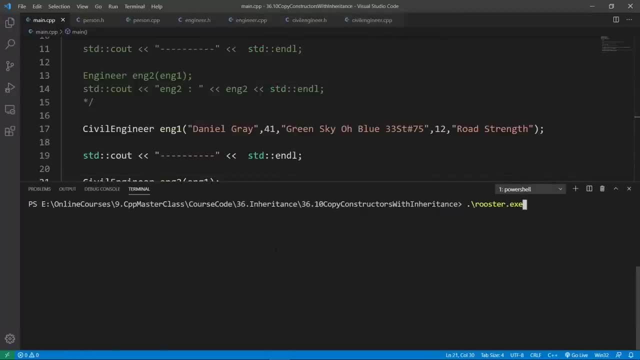 The boat is going to be good, So this is good news. We're going to clear and run rooster and we're going to see that the custom copy constructor is called for person. The custom copy constructor is going to be called for For engineer and the custom copy constructor is going to be called full civil engineer. 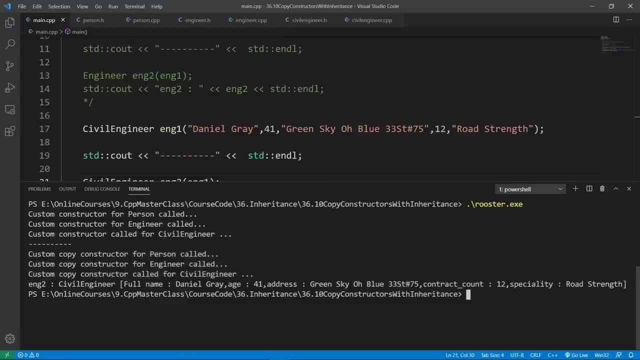 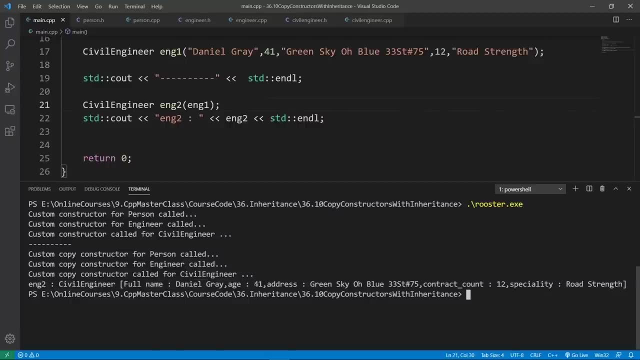 And you see that things are really propagating all the way to the person part And we are calling and reusing our copy constructors And this is really cool. If you go down, you're going to see that the information is printed out correctly. 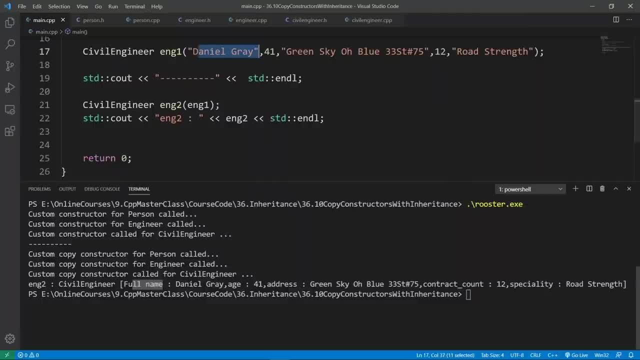 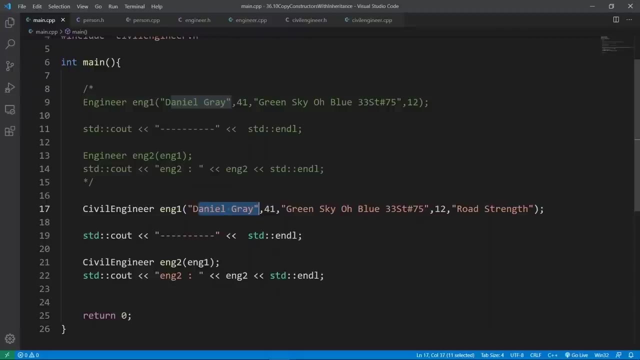 The full name is Daniel Gray, which we have in engineer one. The age is 41. The address is all this gibberish, The contract count is 12 and the speciality is road strength. And we are properly reusing our copy constructors in our inheritance hierarchy. 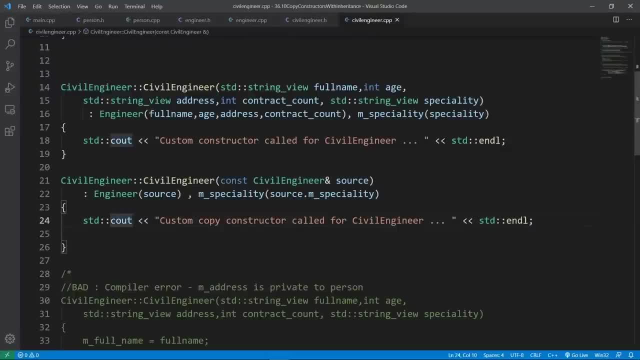 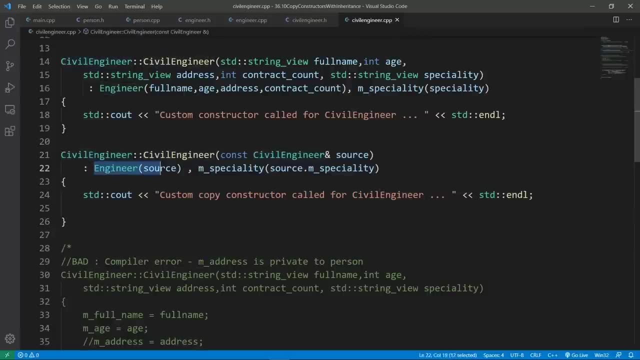 This is really all I had to share in this lecture. Again, the syntax you should be using to set up your copy constructors is what we see here. This is going to be reusing the code we have in our upper classes, in our hierarchy. 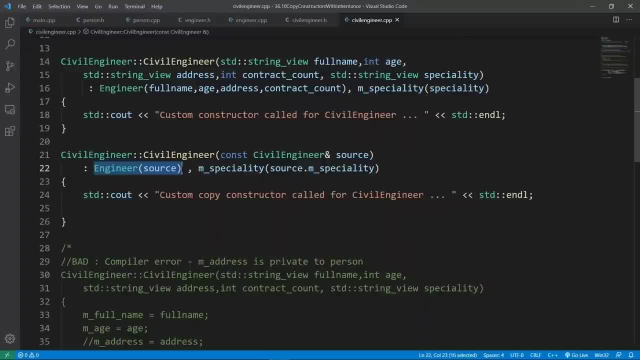 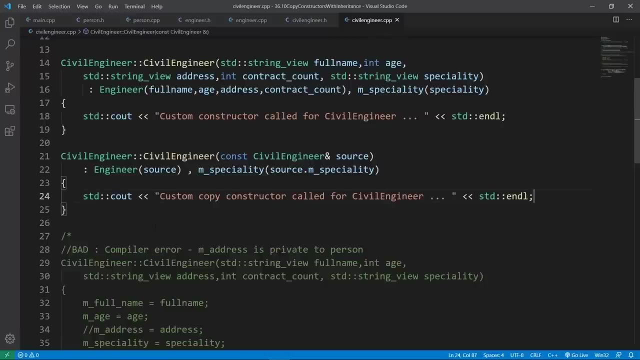 We will be avoiding the temporary copies we saw when we called the other constructor directly, And this is much cleaner. It is reusing code we have in other classes. We are going to stop here in this lecture. In the next one we're going to see that it is actually possible to inherit base constructors. 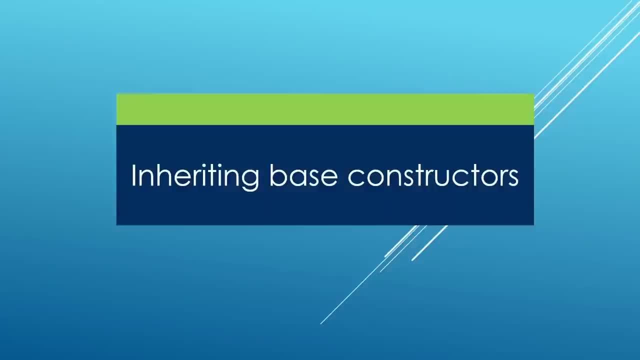 Go ahead and finish up here and meet me there. In this lecture we're going to explore the fact that we can inherit base constructors and use them in our derived classes. We will be reusing the same hierarchy we have been using, So we will have the person class. 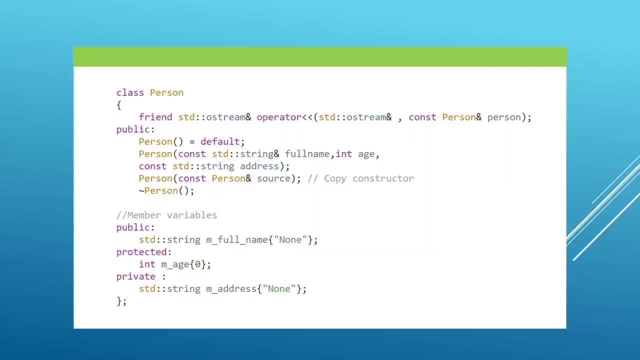 And we will be inheriting from this class, This person, to create an engineer class, And that's what we're going to be using to learn about this concept here. So the person class is what we know from the previous lectures. We have a bunch of member variables here. 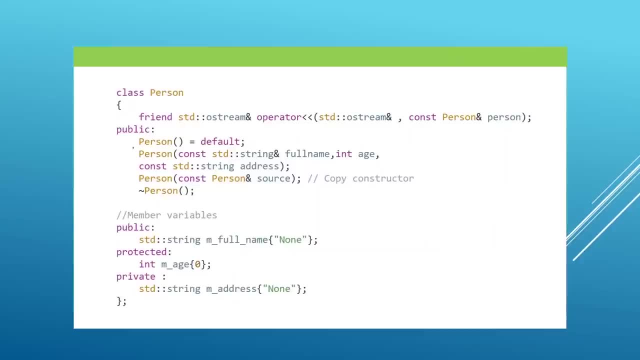 We have the full name, the age and the address And we have a bunch of constructors. now We have a default constructor, a custom constructor and a copy constructor that we set up tirelessly in the last lecture. Now, what do we mean when we say: 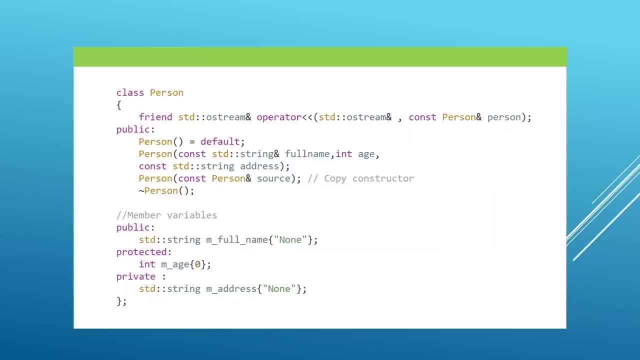 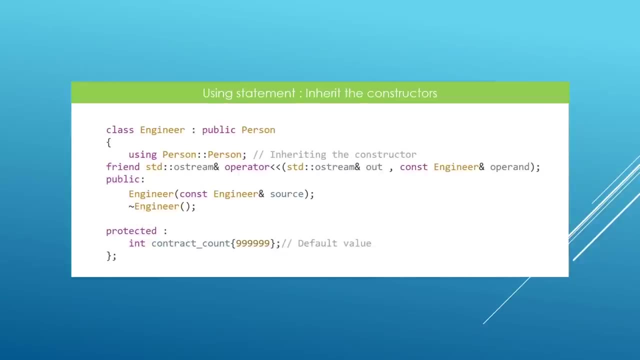 that we can inherit a constructor. Well, base constructors are not inherited by default, And what we mean by that is that by default, it is really not possible to get derived classes to use base constructors to set up things, But it is possible to tell the compiler to use the base constructor to set up our own objects. 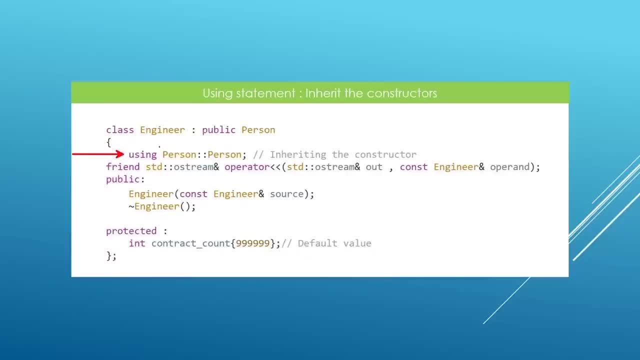 For example, we can put our statement here saying, using person: This is going to tell the compiler: when welding engineer objects, don't use your own constructor. set up a base like a constructor which is going to only initialize the base member variables. 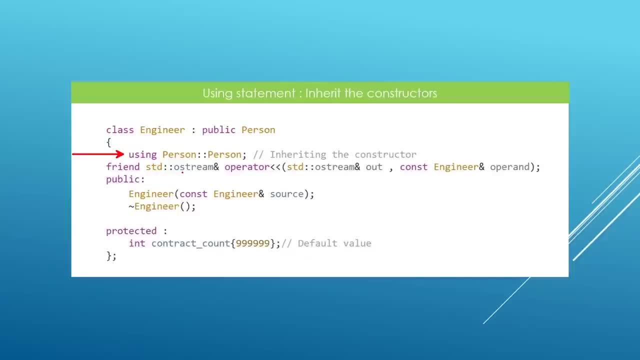 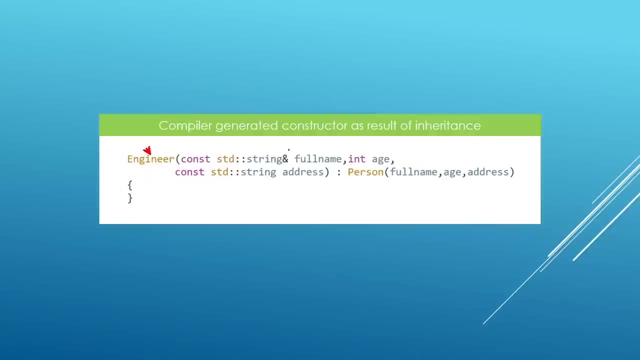 And the compiler is going to see this statement and it is going to generate a constructor for you that looks something like this. So it is going to be engineer. It is going to be taking in the full name, the age and the address. 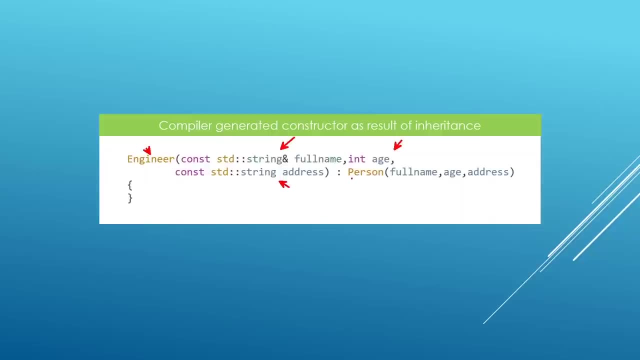 And it is going to be Forwarding the work to initialize your object to the person class, And this is all this constructor is going to do. Hopefully, you can see that this is called inheriting a base constructor, because all this constructor is really doing is initializing the base member variables. 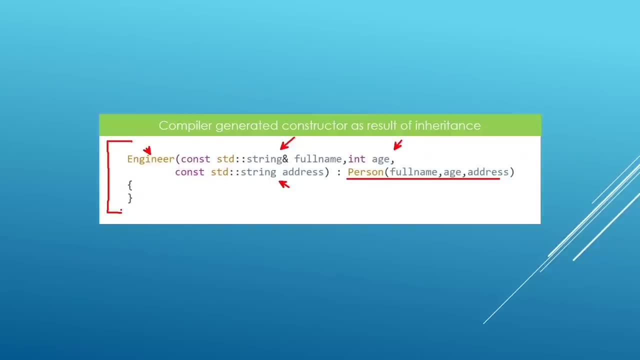 It's not initializing any member variable that belongs to the engineer class. So the engineer part of us is going to be basically empty, containing junk data that we get by just calling the default constructor, and we will only be initializing the data belonging to the person part of us. 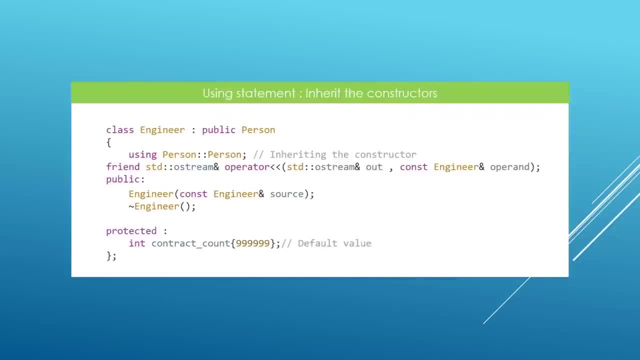 This is really what I want you to see. Again, the syntax is what we see here. This is going to tell the compiler to generate a constructor that is only going to initialize the base member variables, But this constructor will be callable and usable from the engineer class. 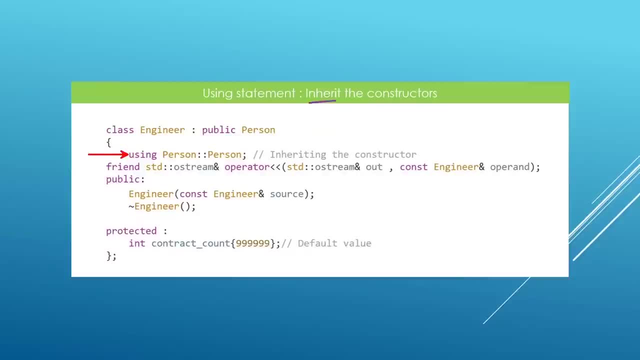 Okay, so this is really what we mean By inheriting constructors. one thing you should know is that the constructor is going to be inherited with whatever access specifier it had in the base class. So if our constructor was in the public scope, it's going to be inherited with public access. 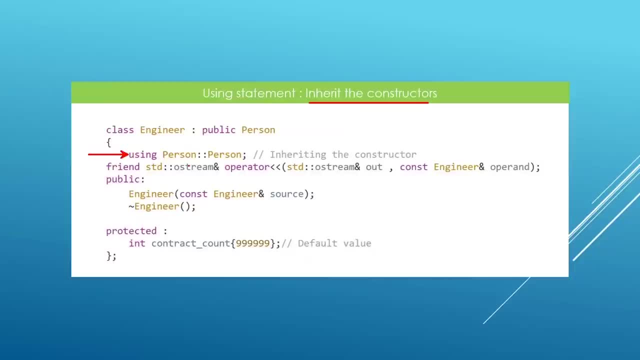 So we will be able to use it from the outside and world engineer objects. If it was in a protected scope, we won't be able to use it from the outside. If it was private, we won't even be able to use it from a derived. 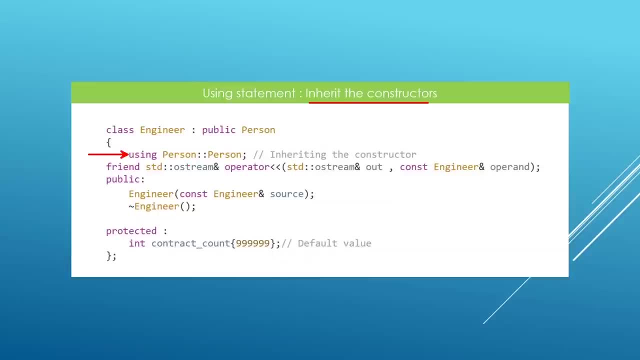 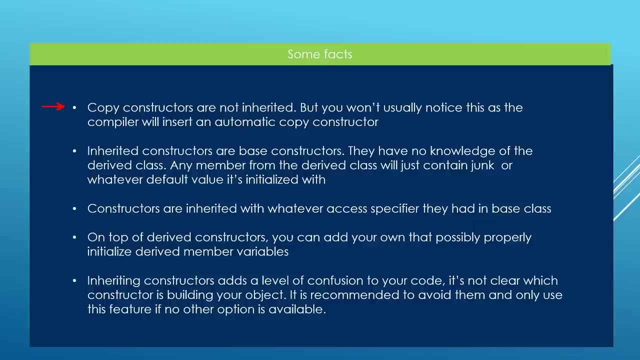 Class. you should really know that. So it is going to be inherited with whatever access specifier we had in our base class. Now that we know this, let's see some things you should really be careful about. The first is that copy constructors are not inheritable. 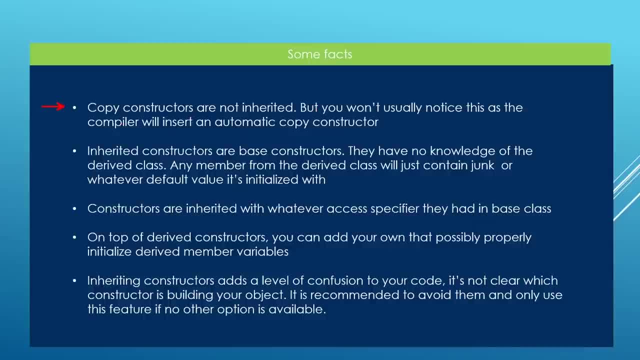 If you're trying to do that, you're going to get a compiler error. But you won't usually notice this because the compiler is going to insert copy constructors for you anyway. This is going to become a problem if you are doing some dynamic. 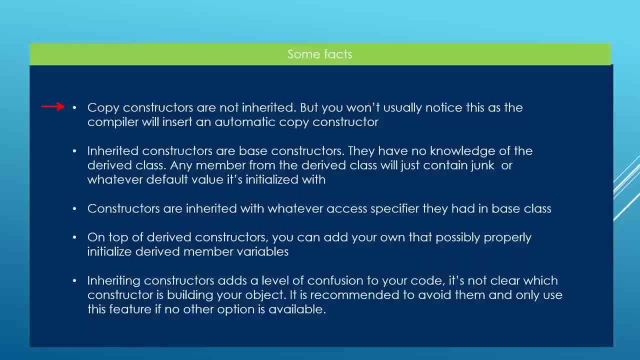 Memory allocation and you're going to get pointers copied. This is really bad. If you don't know about this, please go back to the chapter on classes and you're going to see all the story about shallow copying and deep copying. We talked about these things. 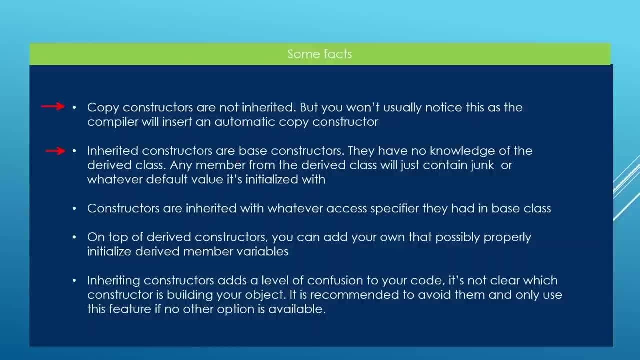 Another thing you should know is that inherited constructors are really based constructors, And what we mean by this is that they will only be initializing the base member variables because they are based constructors. They have no knowledge of Derived Member variables. That's why they only initialize base member variables. 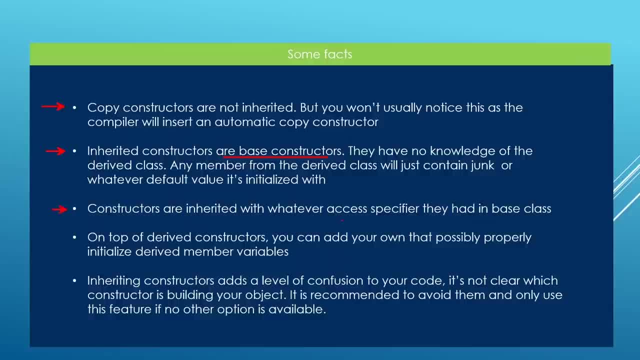 Again, as we say that the constructors are inherited with whatever access specifier they had in the base class, And it is possible to set up your own constructors on top of the inherited constructors and you can use these things. Another thing I should really tell you is that inheriting constructors is going to make your code really confusing. 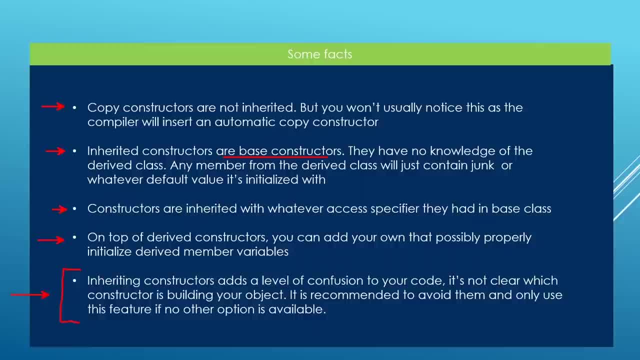 It is a technical possibility, but I strongly advise against using this in your code Because it is just going to confuse people. People are going to see, for example, an engineer constructor and they are going to think that that constructor is going to even initializing the engineer member variables. 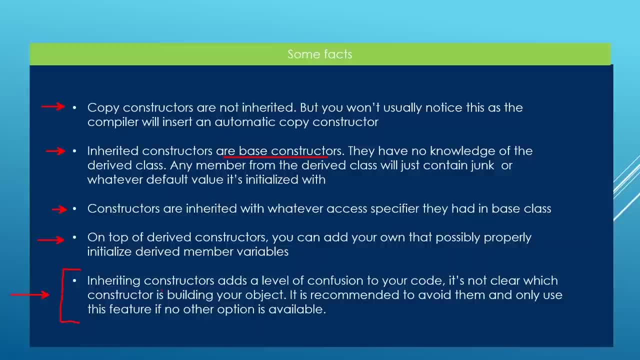 But it's not going to do that because it is a base constructor. It's only going to be initializing the base member variables and that may lead to some confusion or even really bad problems in your code. So don't use this. It is just going to make things confusing. 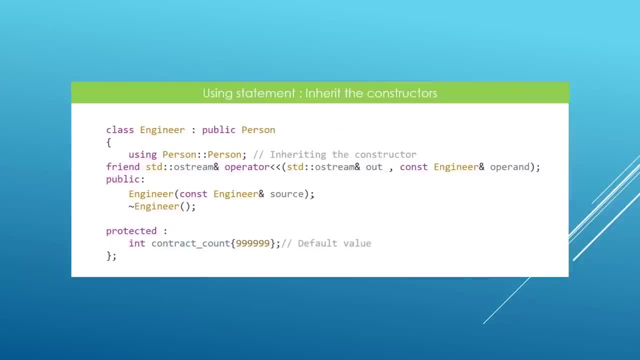 But I wanted you to be aware of This and if you see this kind of set up in classes out there, you will know what they mean. This is just going to inherit a base constructor and use it to build objects. Now that we know this, we're going to head over to Visual Studio Code and play with us a little more. 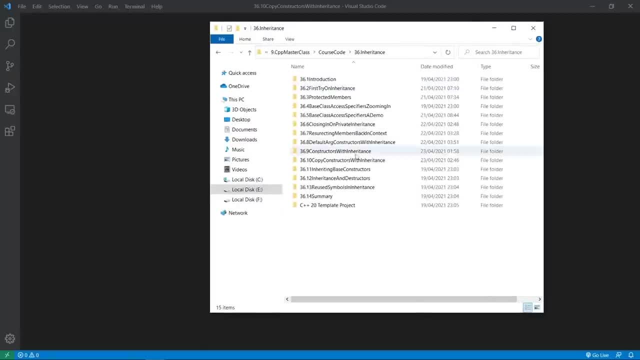 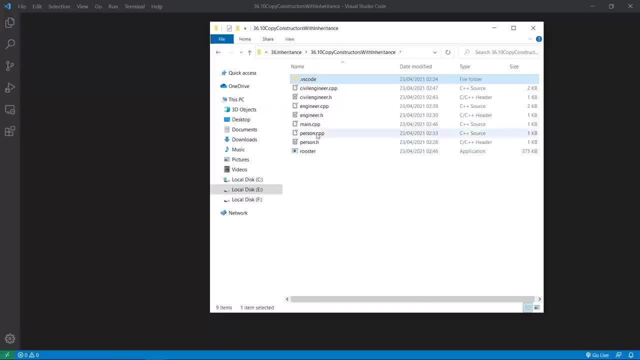 Here we are in our working folder. The current project is inheriting base constructors. We are going to steal code from the last lecture and we will be using the main CPP file, the person class And the engineer class. This is just going to be enough for our purposes here. 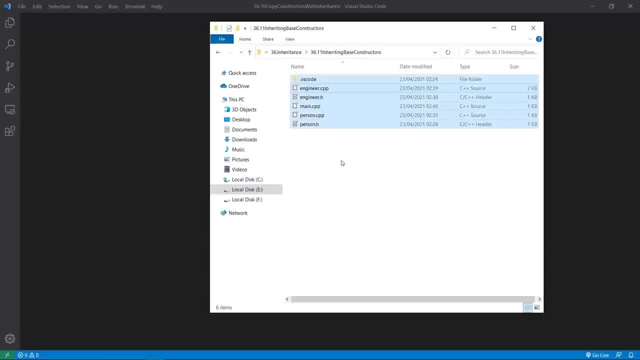 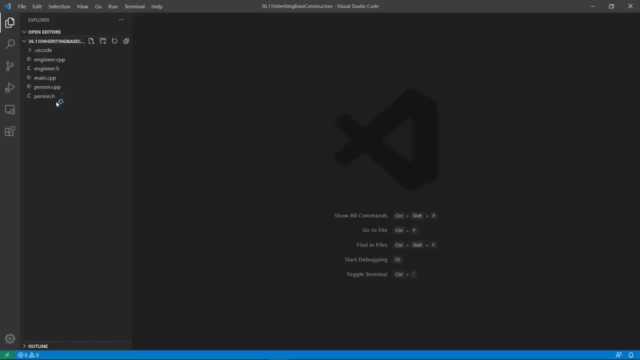 We're going to go back in our current project and we're going to put this in and we will open this in Visual Studio Code by dragging and dropping here. This is going to give us our fun and let's go to person and see that we have our constructors and we have a default constructor. 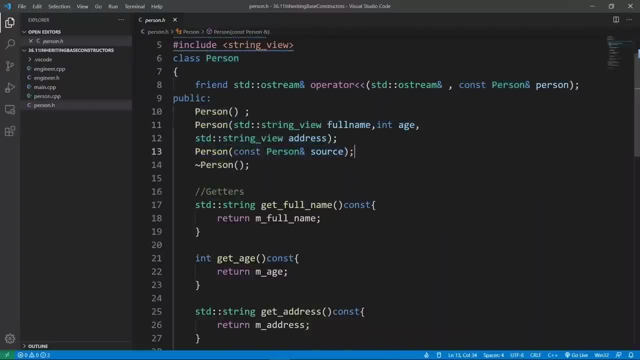 We have a custom constructor and we have a copy constructor. One thing you should know is that copy constructors are not inherited, So you will need to set up your copy constructors explicitly if you want to use them. Note that they won't be coming from the upstream class. 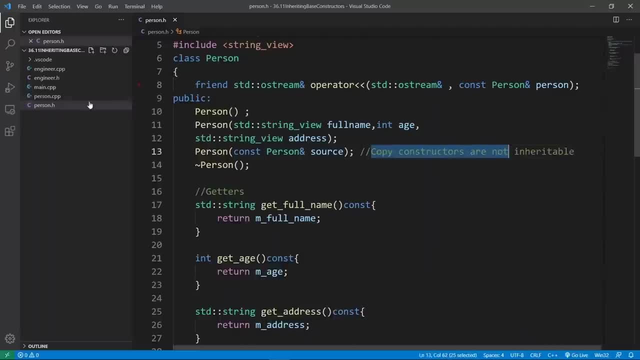 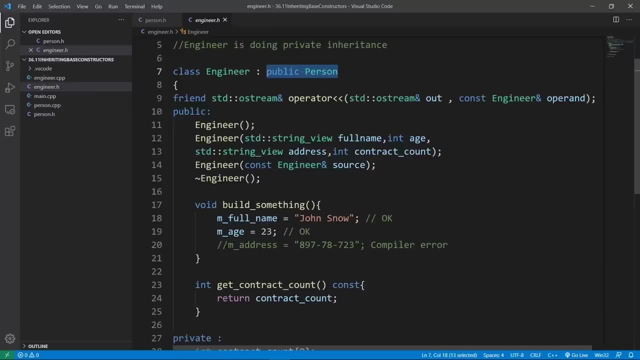 You should know that. OK, so this is the message here. Now let's look at our engineer class. The engineer class is publicly inheriting from person and it has a bunch of its own constructors, But what we want to do is to take out all these constructors, and we're going to take them out. 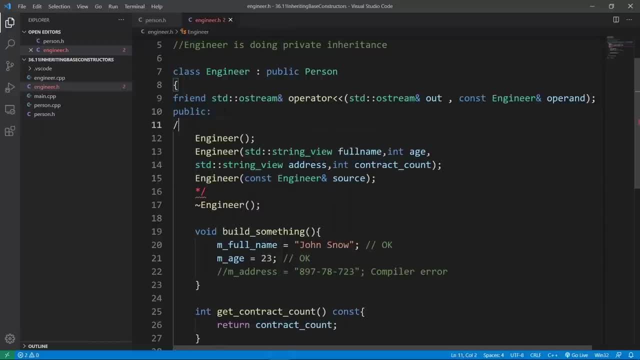 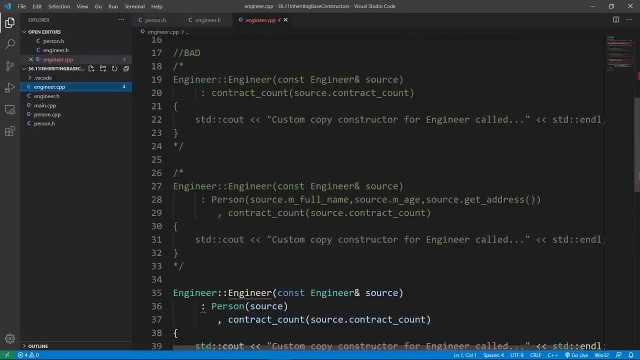 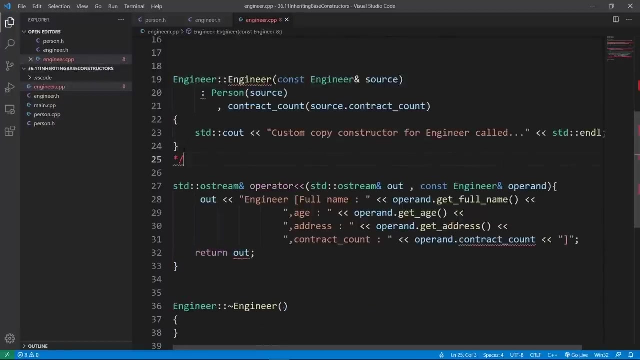 I think We can. Yeah, we're going to take them out. Let's do that, and we're going to go in our CPP file and also take out all these constructors here. We're going to comment them out. I think we can take out all these bad code we got from previous lectures and we're going to just comment out our constructors. 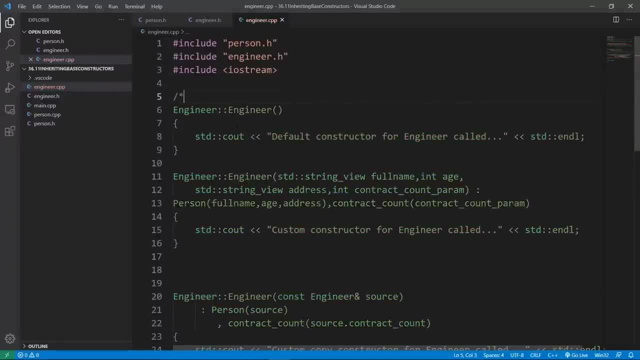 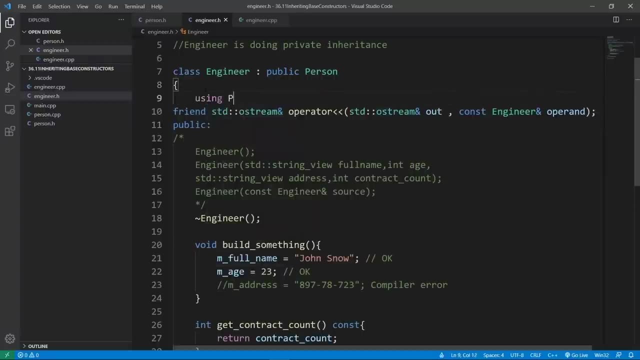 We're going to close them all with a block comment and what we are going to do in our class is say: using person person. We're going to say using person person. This is going to Inherit the constructors from person and now that we have this in place, the compiler is really going to generate a base like a constructor in our engineer class. 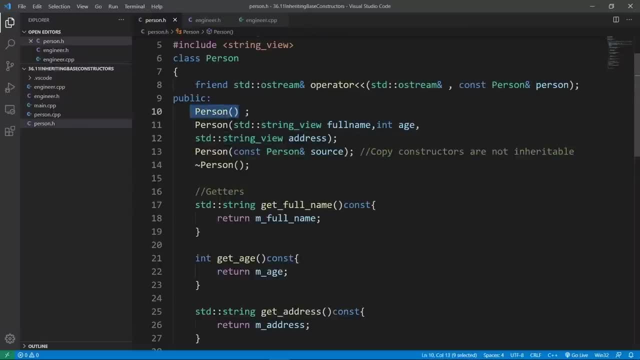 In other words, we're going to have a default engineer constructor which is just going to not initialize anything. We are going to have a custom constructor which is going to take three parameters, but it is going to be an engineer constructor and let's prove this. 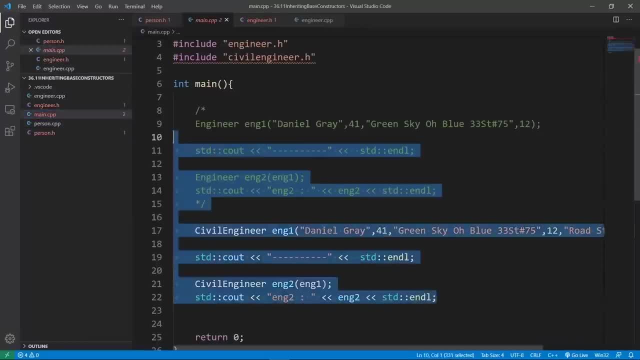 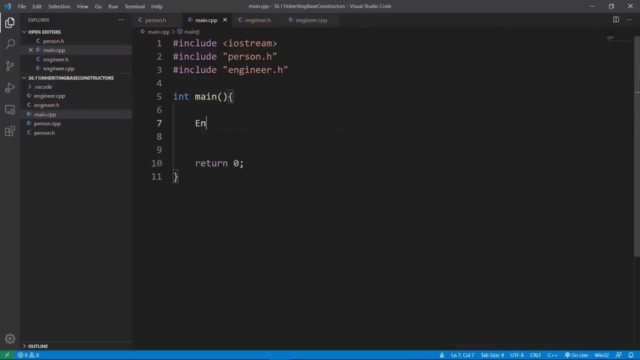 We're going to go in our main CPP file and we're going to take out everything We have here and we don't have a civil engineer file, so we shouldn't really include that. and we are going to create an engineer object We can say, and one using the default constructor. 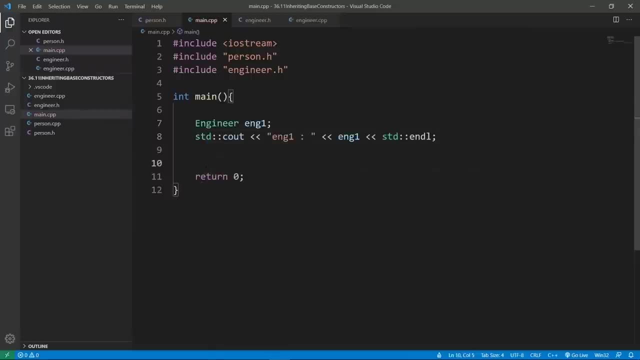 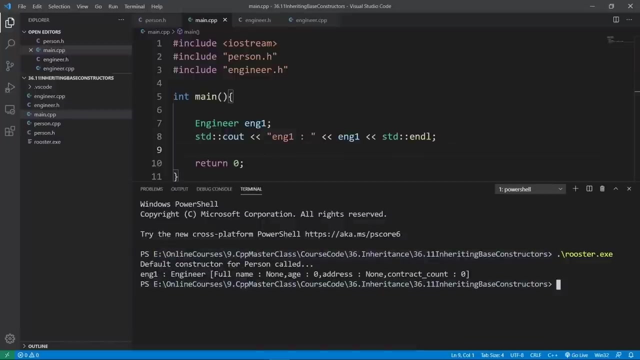 We can try and print that out and you're going to see that this code seems to work in a vicious video code. We can try and build this. We're going to pass this through GCC and we are going to set up a PowerShell window we can use to run and see things, and we're going to see that the default constructor for 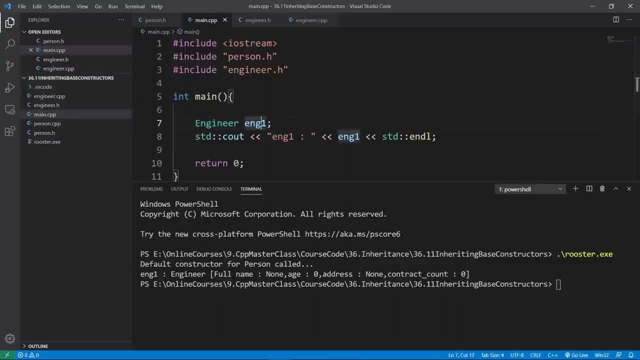 Person, Person was called to initialize this guy and the data is really junk data we have in person. So what the compiler is really doing behind the scenes is to generate a base like constructor at the engineer level, and it is going to call the base constructor to initialize the person. part of us. 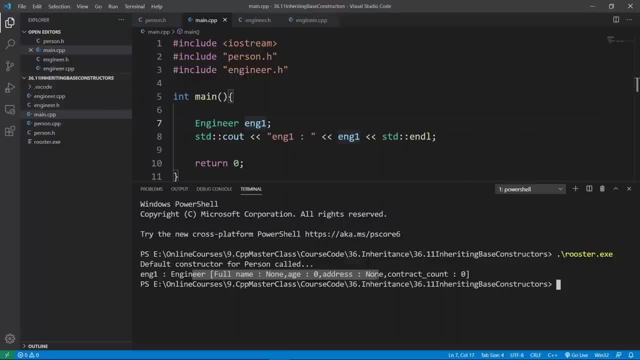 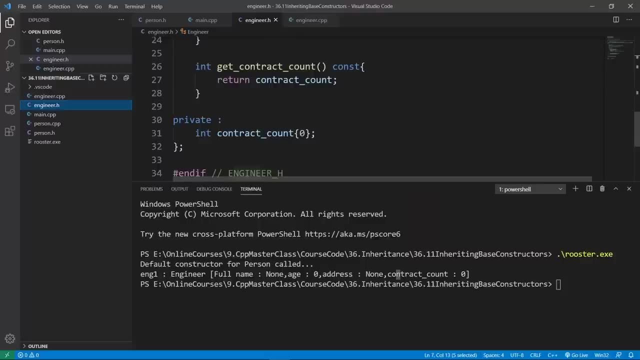 So the data is just going to be junk data we have in person and you're going to see that the contract count is going to be zero. This is just a default constructor which is just going to Grab Whatever defaulted data we have in our object. 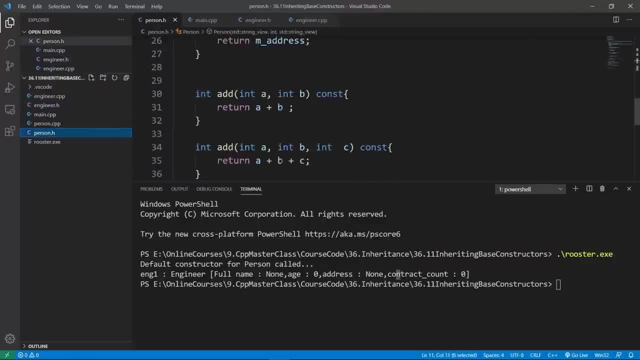 You see, the contract count is zero. If we go back in person, we're going to see that the full name is none, which is what we see here. The age is zero and the address is none. This is a default constructor, but we can even explicitly pass in the data and that's going to also work, so we can pass in the full name, to be Daniel Gray. 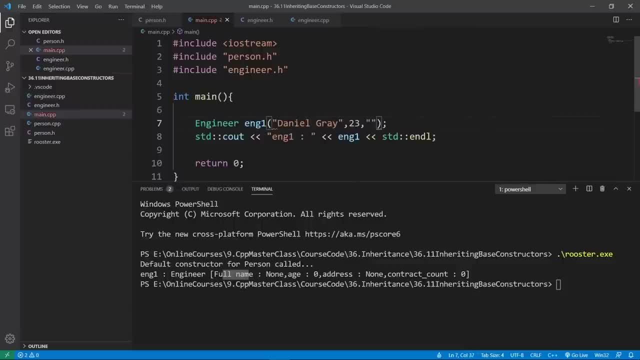 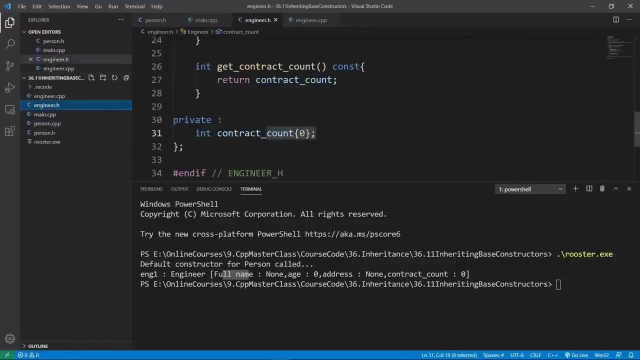 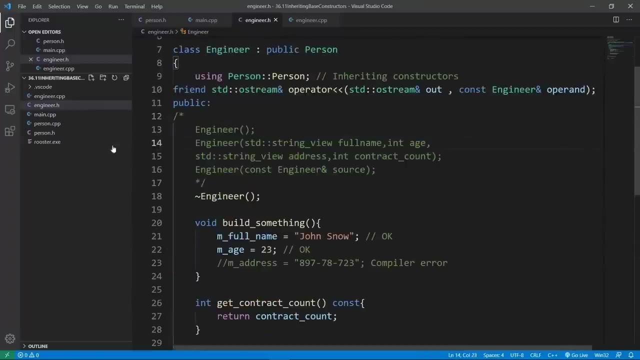 We can pass in the age to be 23, for example, and we can pass in a junk address. let's say something like this, and you see that this is Going to work. Even if we don't have any engineer constructor that takes three parameters. let's go back and you're going to see that all our constructors are commented out. 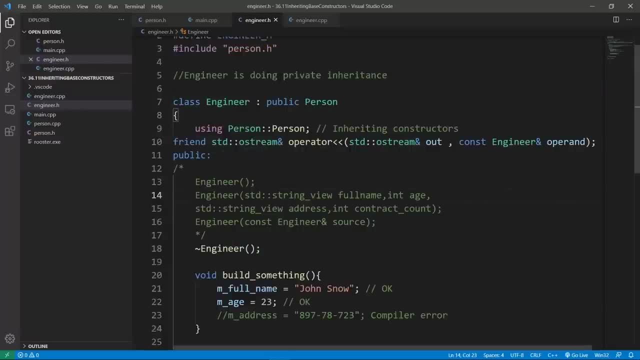 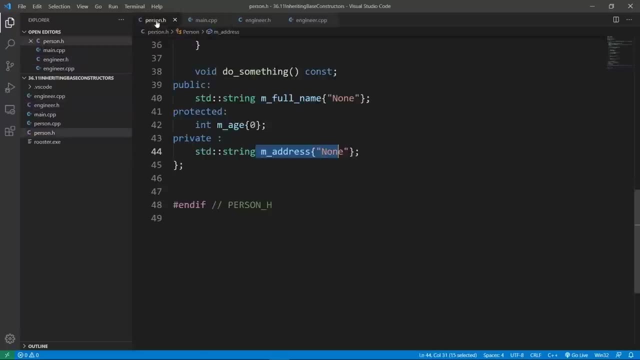 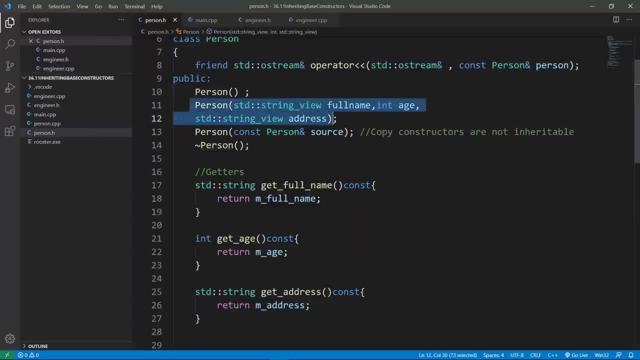 But this is working because we told the compiler to generate a base like a constructor for our engineer, So it is going to also have an an engineer constructor that looks like this constructor here, which takes in three parameters. this is really cool and this is really crucial to understand. so, again, we are going to set up a 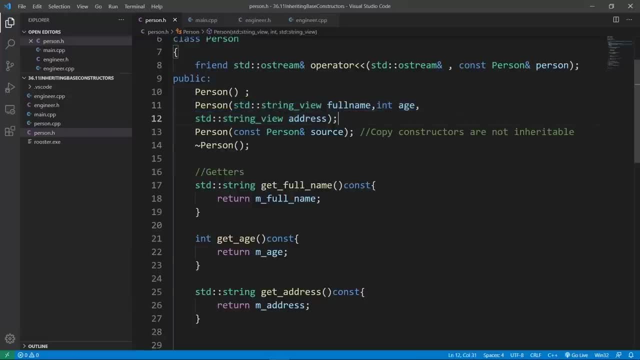 constructor for engineer. so it is going to be an engineer constructor, but it is going to be taking three parameters, just like the person constructor here, and this is the message i really want to convey here. so if we run this code, you're going to see that it is going to work. it is going to call. 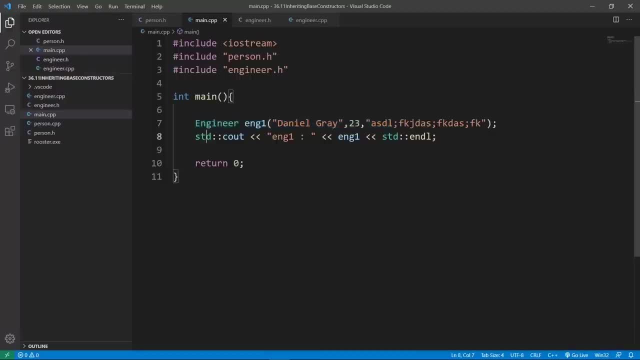 our base like constructor for engineer and we're going to have the data forwarded. n, but you're going to see that the contract count is not going to be taken into account, so it is going to still contain some default data. if we try and pass that n, we're going to see that we're going to get a. 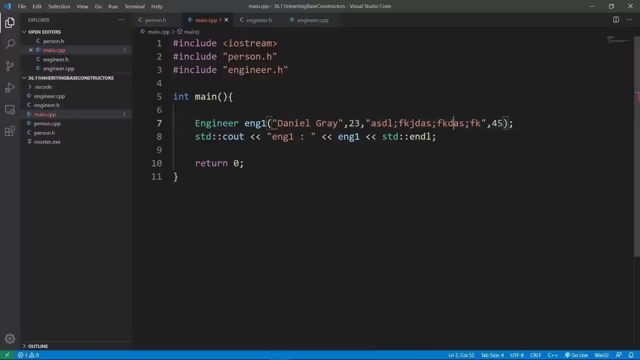 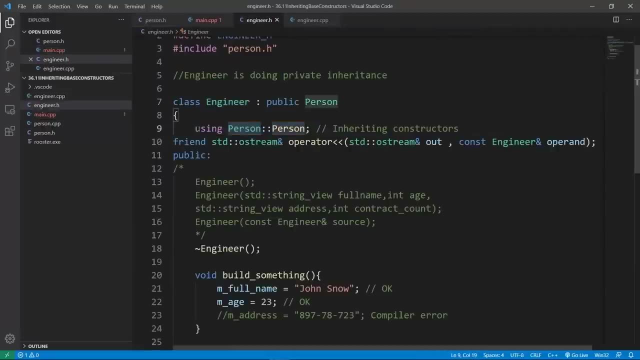 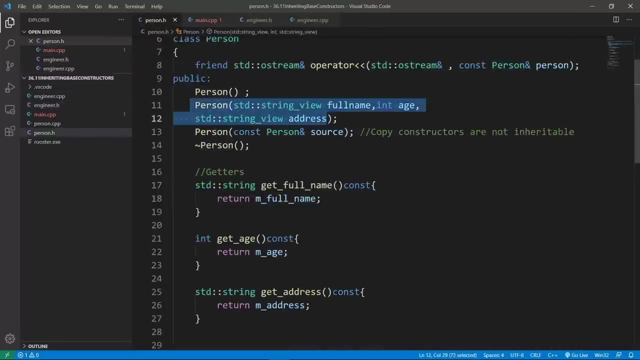 compiler error, because now we have no such constructor that takes four parameters. the only one we have is one that is generated because of this statement here, and this is going to be a base like constructor, which is just going to take three parameters, just like this constructor here. 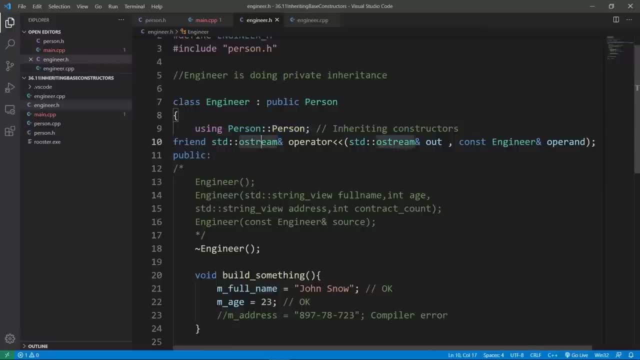 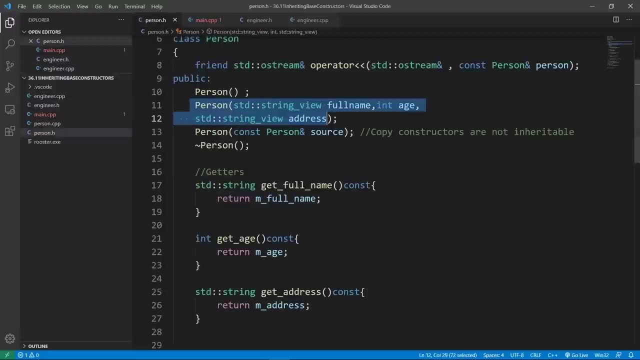 and another thing I don't think I made clear enough is that this is going to bring in all the constructors you have- notice that we just put in this statement- but it is going to grab all these constructors we have, except for the copy constructors which are not inherited in c++. so you should really know this. 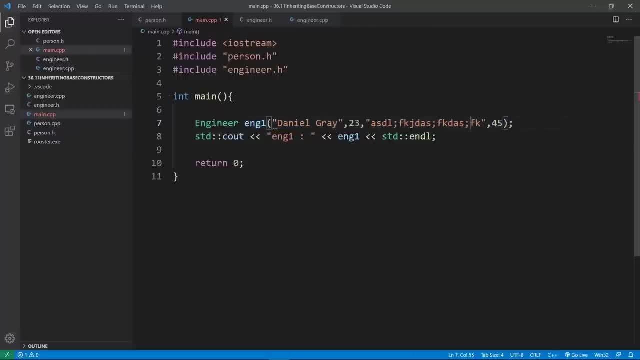 if we build this code, we're going to get a compiler error because the compiler wants to know what to do with the 45 parameter that we have here. but let's build and really show you this. you need to see this compiler error with your own eyes. let's go in, so the world is finished. 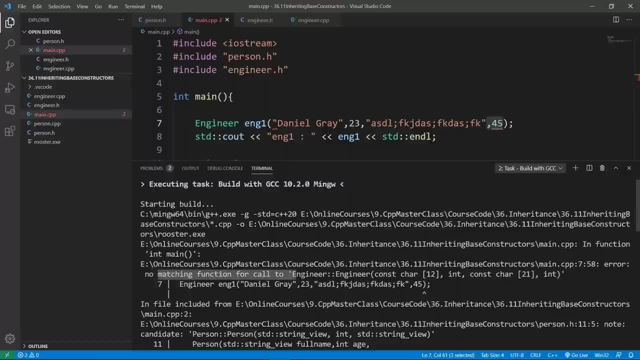 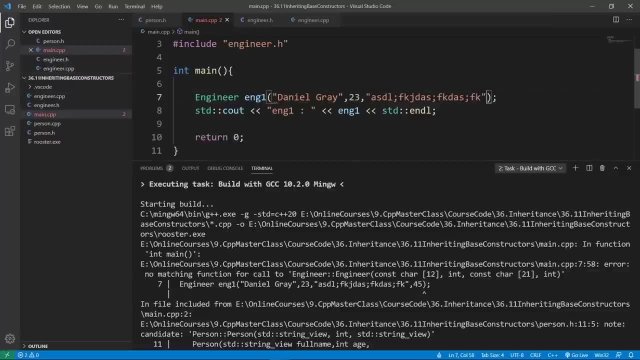 with errors and we have an error saying no matching function. call to this constructor, which takes four parameters. if we take this out, we're going to see that this is going to work. this is going to use the compiler generated constructor. as a result of this statement, we 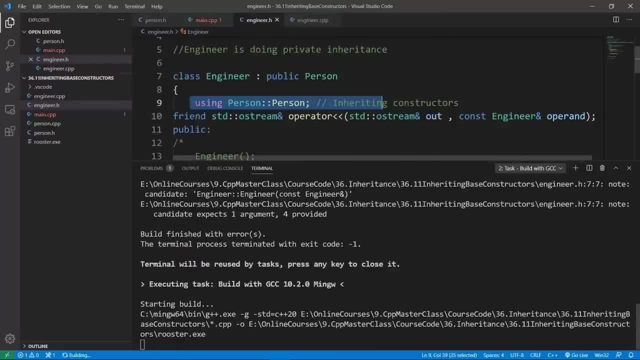 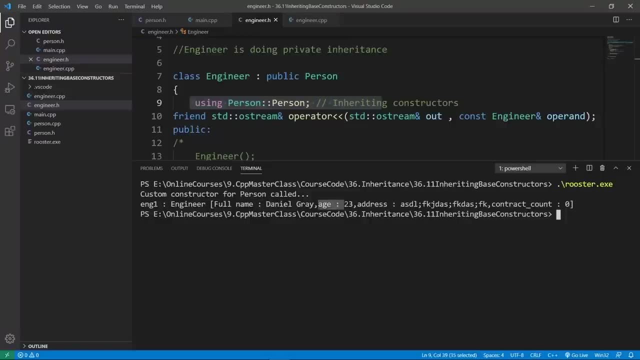 have in our code now, if we build, we're going to see that this is going to work. okay, the build is good, we can clear and run. we're going to see that we have the full name to be daniel gray. we have the age to be 23. 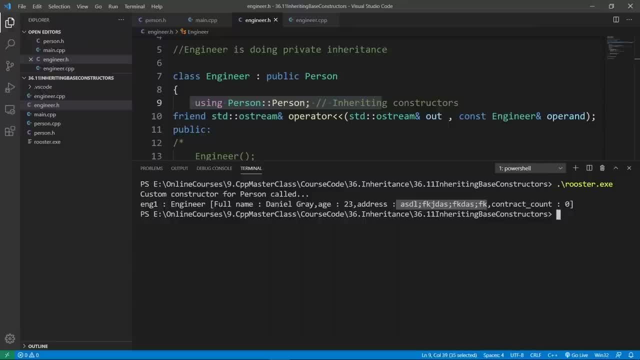 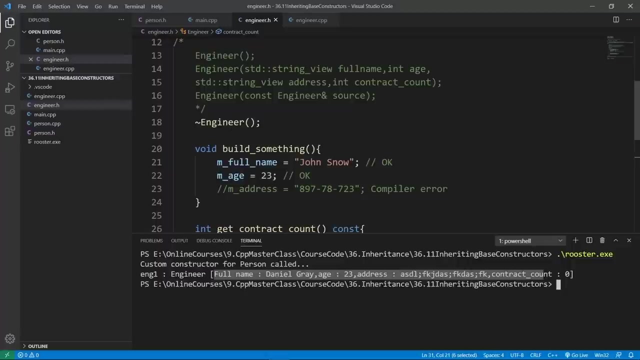 we have our address, which is really some junk data, and the contract count has no data and it is just the default data we have in our member variable. here we have no way to initialize this from a base like a constructor. but not everything is really bad news if you don't want to be limited. 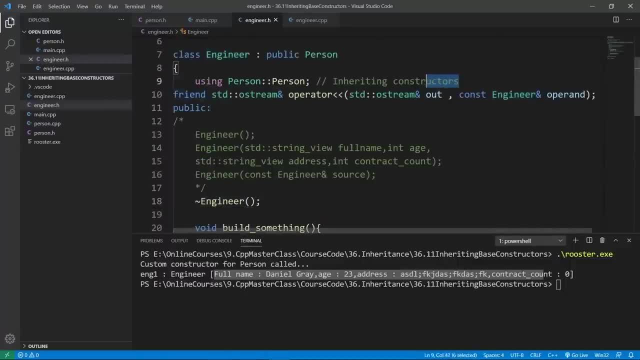 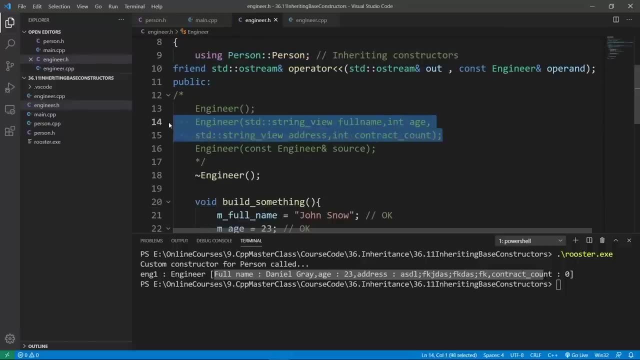 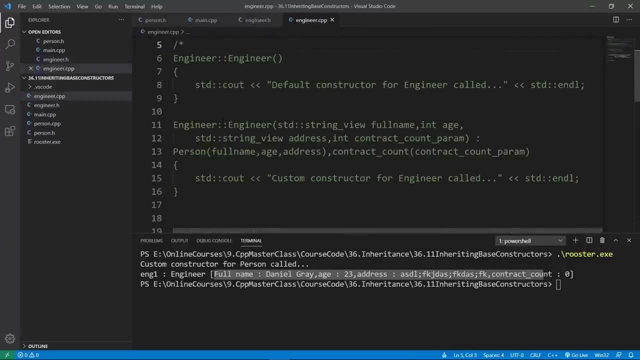 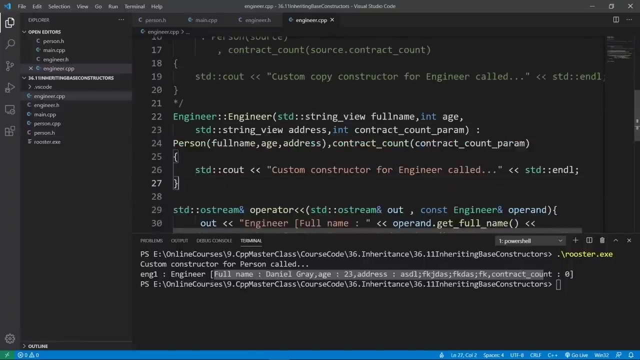 by the constructors that are generated by your compiler as a result of inheritance. you can up your own constructors. for example, we can uncomment our engineer constructor here and bring it out of our comment. we can do something like this: we can go in the implementation file and also bring this out of our comment section, and now we will be able to use this constructor. 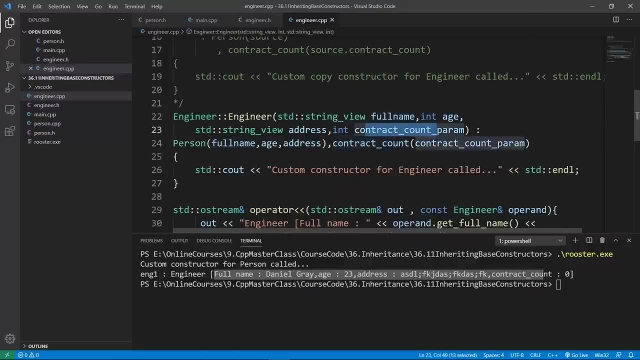 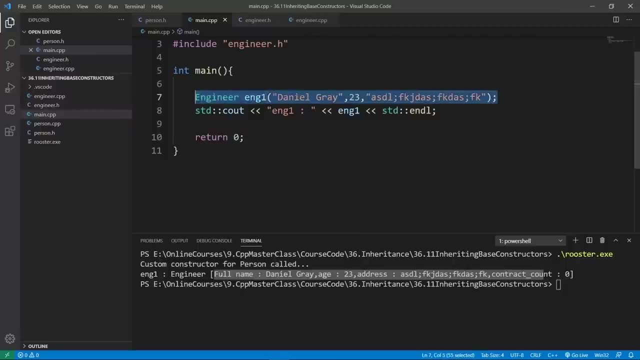 which is going to take the fourth parameter here and do something with it. now, if we go back in main, the code with three parameters is going to work. it is going to use the compiler generated constructor, but if we pass the contract count to before, this is also going to work, because it is 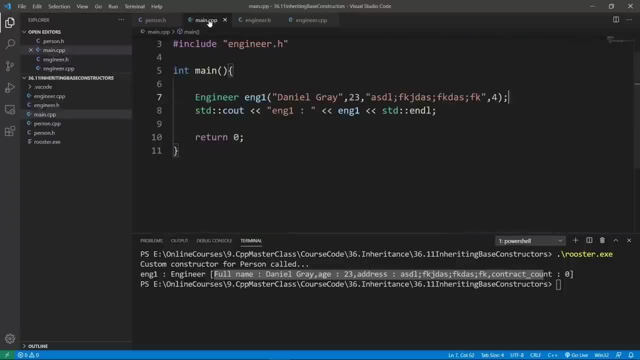 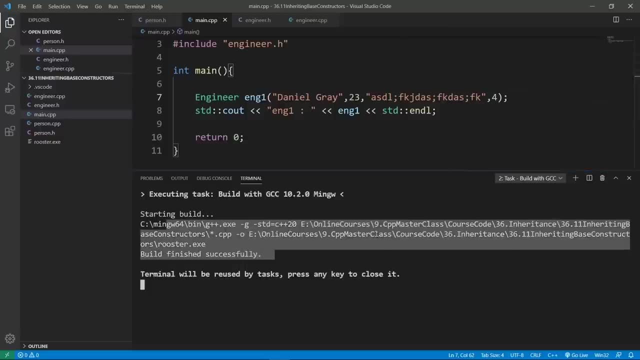 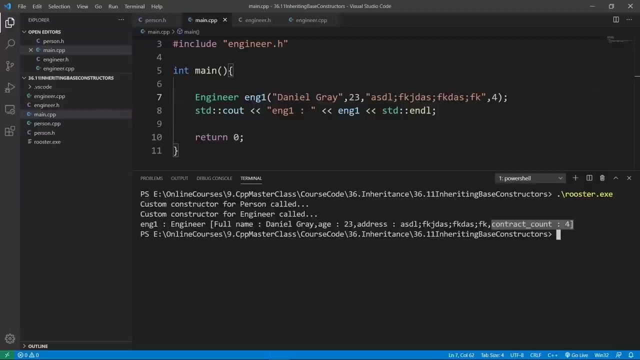 going to be using our own constructor here. if we build the code, we're going to see that it is going to work just fine. let's use gcc to show this. you're going to see that the world is good. we can clear and run rooster. now our contract count is taken into account and this is really cool. 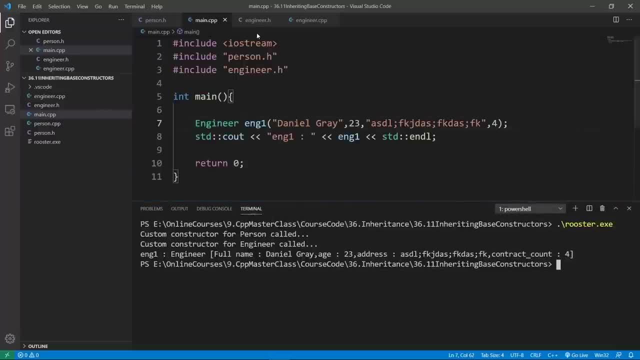 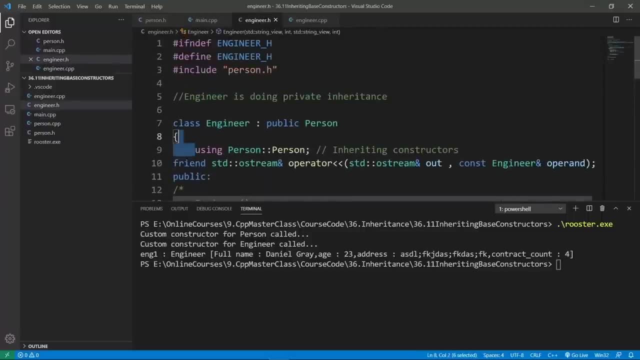 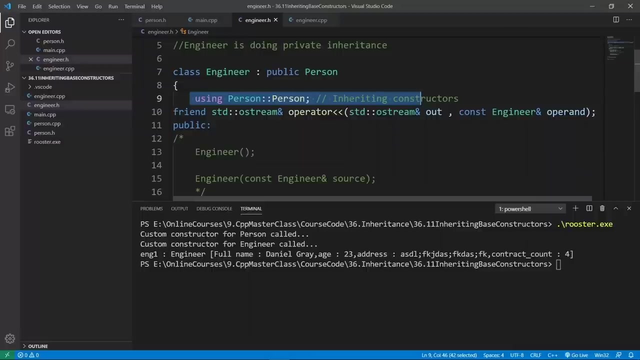 this is really all i wanted you to see in this lecture: that you can let the compiler generate the base like constructor using the syntax we have in our header here. this using statement can really show up anywhere, but it is going to inherit the constructor with whatever access specifier: the 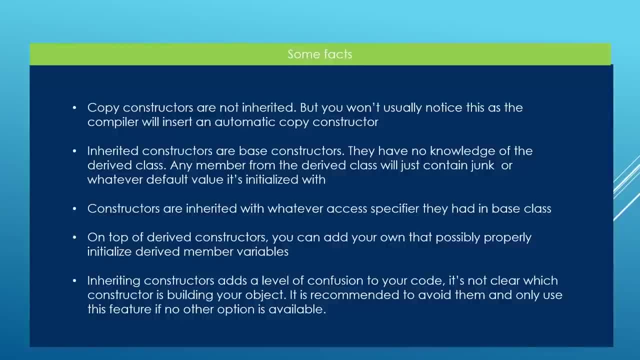 constructor had in the base class, and you should really keep these points in mind, especially the last one that inheriting constructors is going to make your code confusing. people are going to notice that they can call constructors that are really not going to be initializing derived member variables, and this may cause 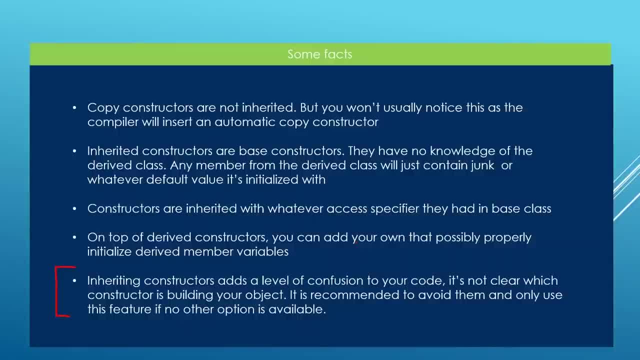 serious problems in your code. we are going to stop here in this lecture. in the next one we're going to explore how inheritance works with these structures. so far we have been ignoring the structures. we are going to focus on them in the next lecture. so go ahead and finish up here and 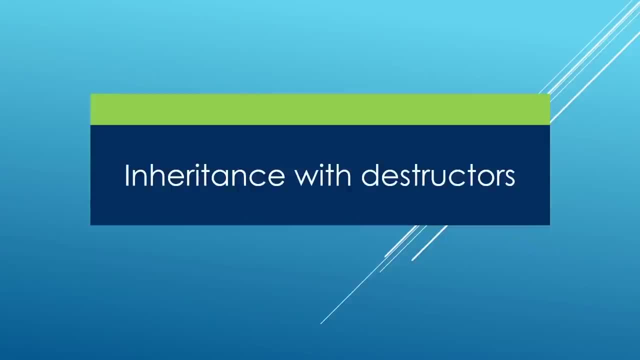 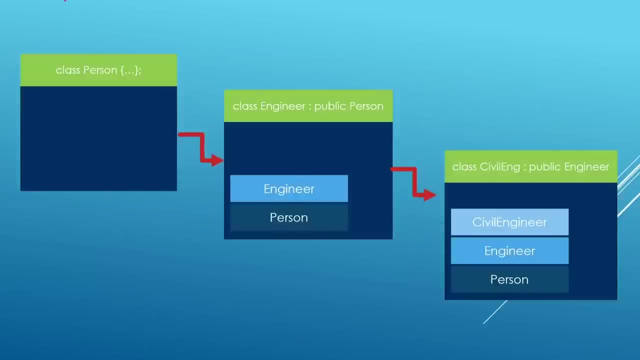 meet me there. in this lecture we're going to focus on how destructors work with inheritance and suppose we have an inheritance hierarchy, like we have been using all along in this chapter. so our base class is person. we have the engineer class which is publicly inheriting from person. 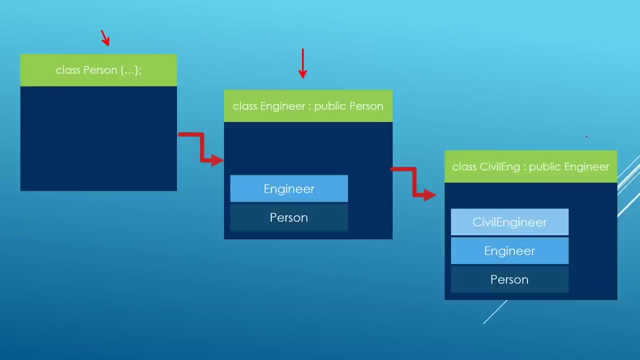 and we have a civil engineer class which is inheriting from engineer publicly. so when we create the civil engineer object, we have seen that the burst part is built first. so we are going to build the person part of us. we are going to build the engineer part of us on top. 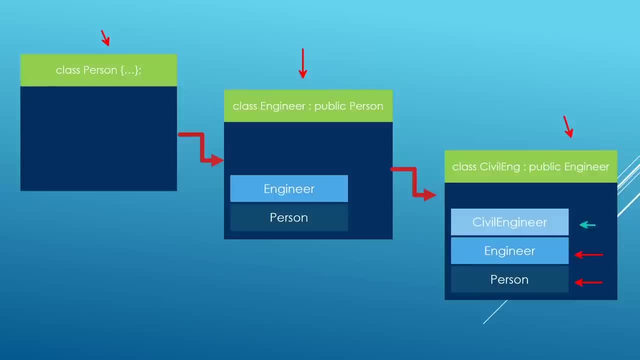 of that and we are going to build the civil engineer part of us on top of that. so the constructors are going to be called in this order. we will call the person constructor first, engineer constructor after that, and then a civil engineer constructor after that to set up our civil 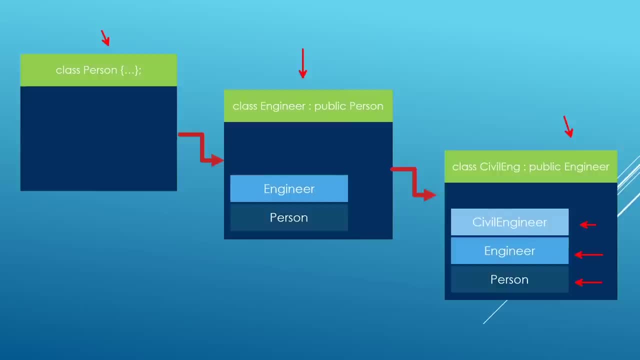 engineer object. the thing i want you to see in this lecture is that the structures are called in the reverse order to that, so the most specialized destructor is going to be called first, then we're going to destroy the engineer part of us, and the person part of us is going to be destroyed last. 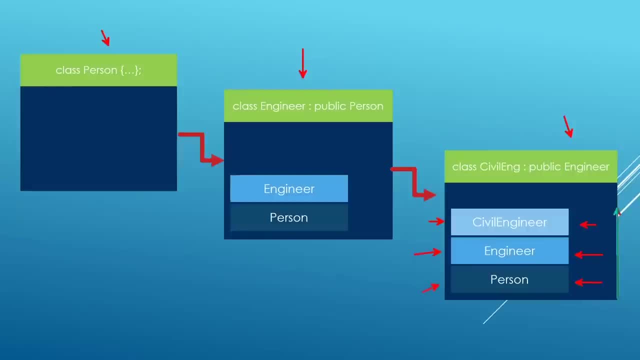 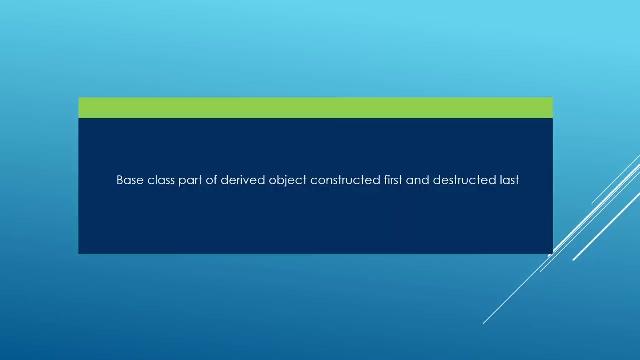 so we are going to construct things in this order, from the base part to the most specialized one, and then we are going to destroy things in this order. so the structures are going to be called in the reverse order than the constructors. that's the message i want to convey here, and we're going to 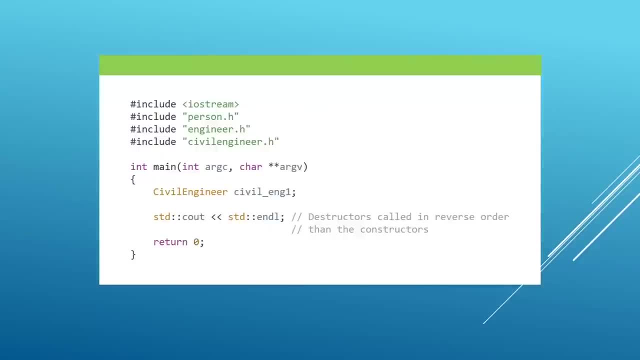 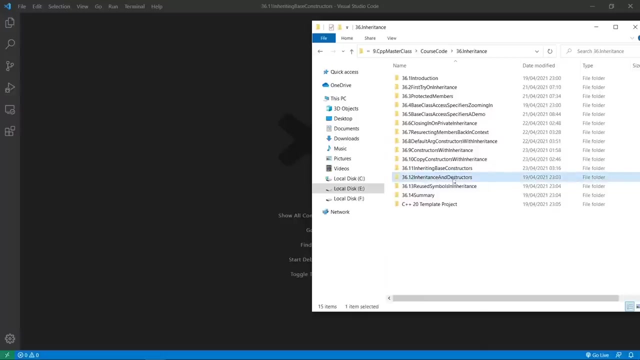 set up a simple example to play with us. we're going to create a civil engineer object and we're going to see the order in which these things are called. and let's head over to visual studio code and actually do this. here we are in our working folder. the current project is inheritance and destructors. 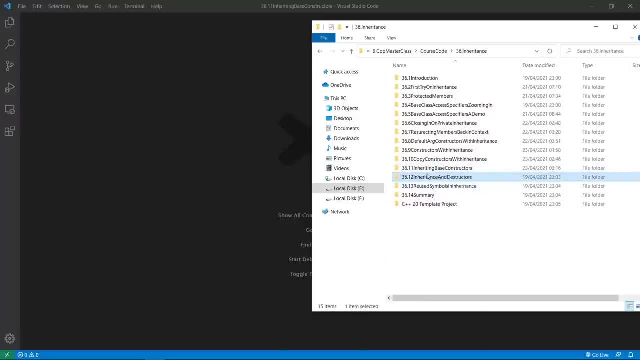 we are going to be reusing the code from a previous lecture. i don't think the last lecture is a good example because we don't have a civil engineer class, so we are going to go to the lecture before that and use the code from our lecture or the copy. constructors with inheritance. 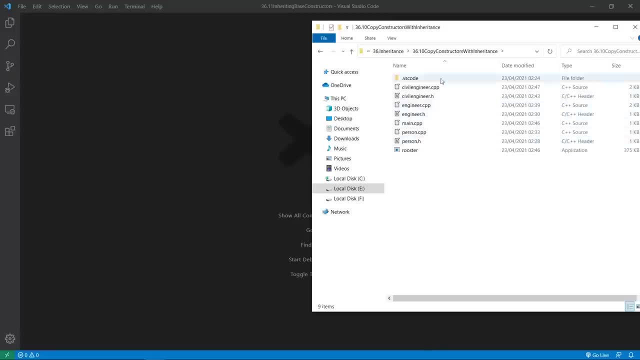 that's going to give us all the classes we have- person engineer and civil engineer- and we need that in this lecture here. so let's grab all these things. we're going to copy them and put them in our current object, which is inheritance and destructors, and we are going to open this in 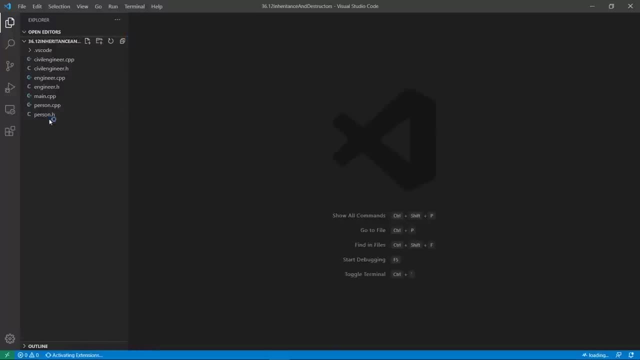 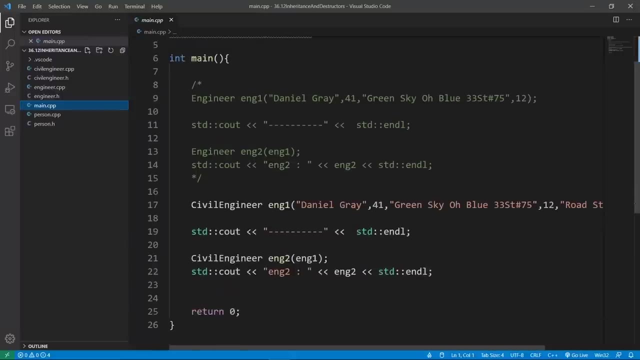 studio code and it is going to be our starting point here. so we have person engineer and civil engineer. let's see what we are doing and the main cpp file. we can take out all the junk here or we can leave in the civil engineer object we are creating here and we're going to see how. 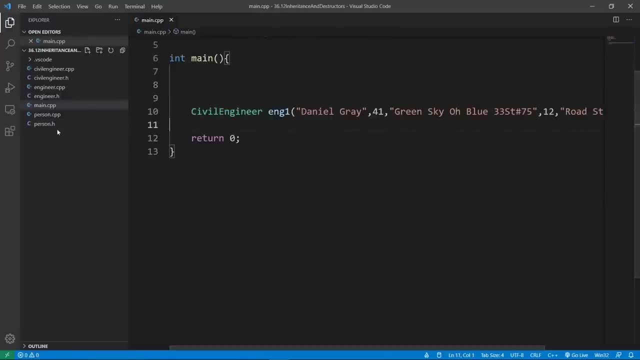 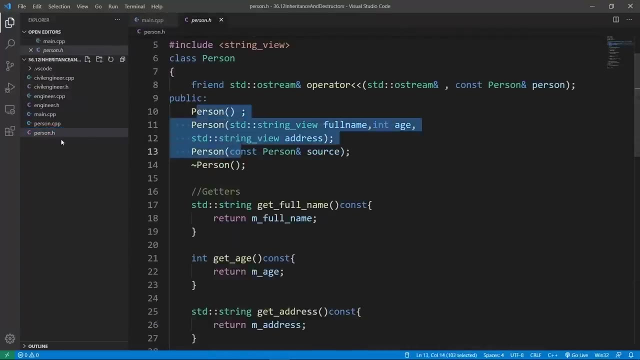 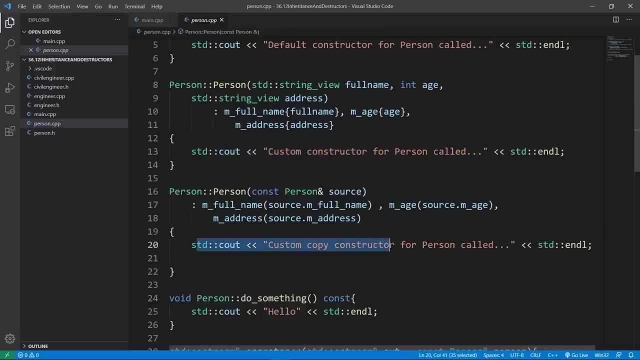 the constructors and destructors are called. we're going to go to person and make sure we have a constructor and we have a bunch of constructors and let's go to the cpp file and see that we have messages in our constructors. this is really what we expect, but we 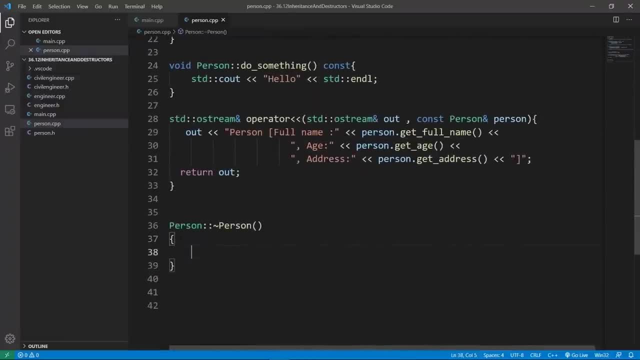 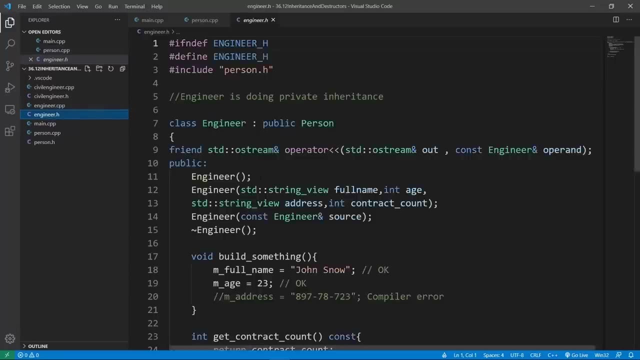 want to also put a message in the destructor. let's say stdc out and say destructor for person called. this is going to do. we're going to go in our engineer class. we're going to see that we have a bunch of constructors, we have a destructor here. we're going to hop over in the cpp file. 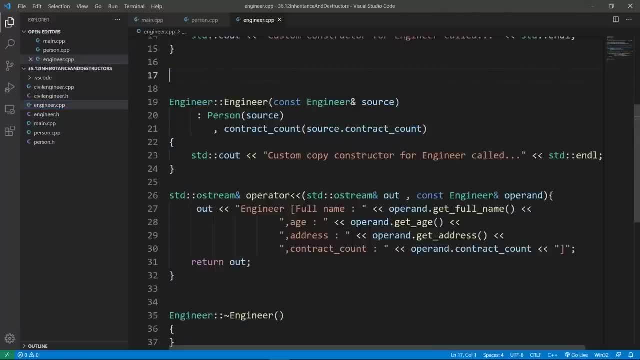 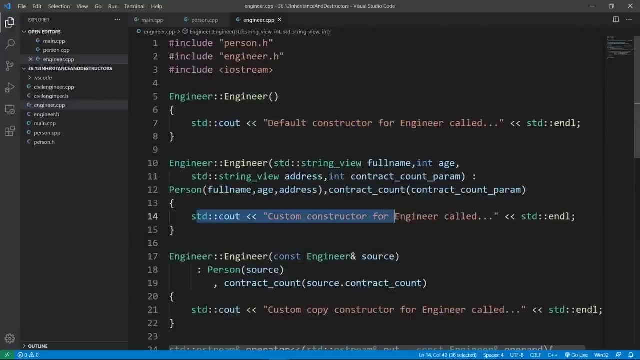 and make sure we take out the bad code here, because we don't really need that, we only need good code- and we make sure that we have output statements in our constructors to know when they are called. looks like we are good. we're going to put an stdc out statement in our 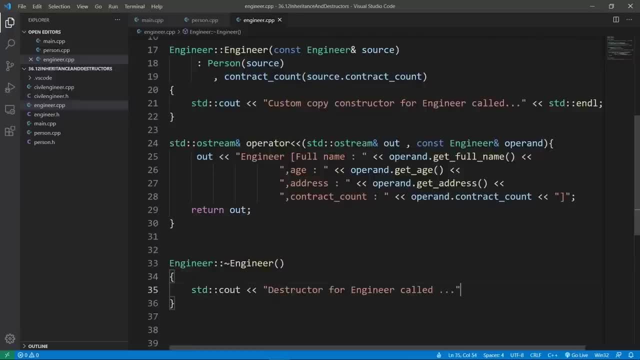 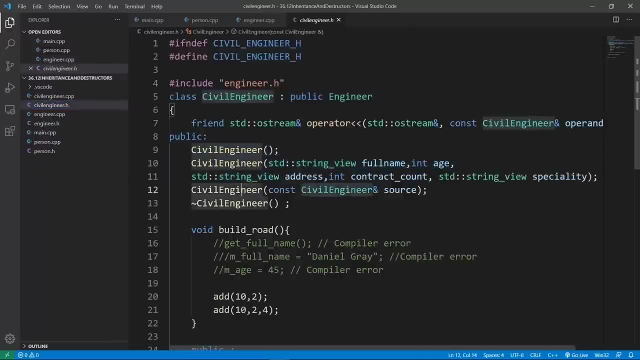 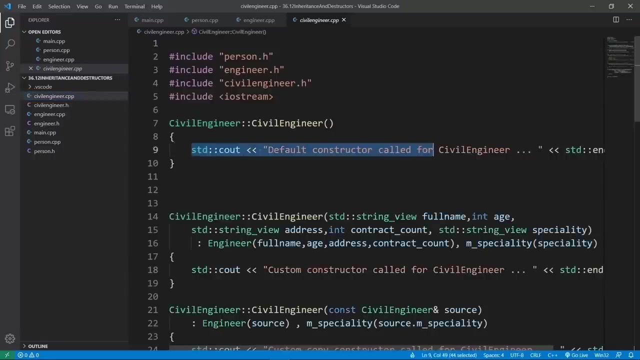 destructor for engineer, or engineer called. this is going to do and we are going to hop over in our civil engineer class. we're going to have a bunch of constructors. we're going to have a civil engineer destructor. we can go in the cpp file and make sure that we have. 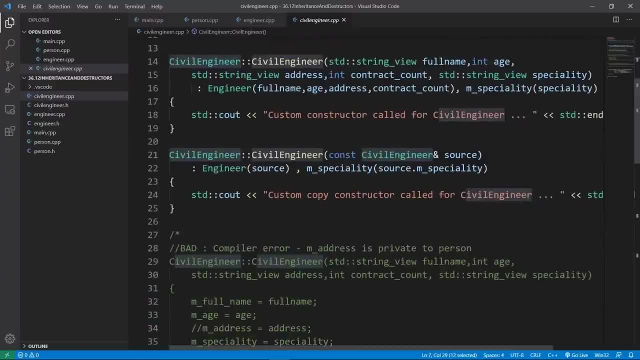 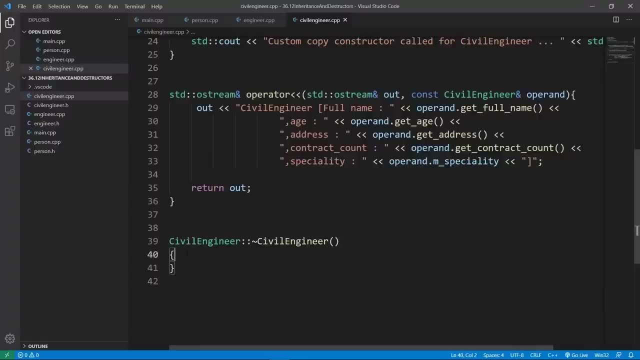 output statements in our civil engineer constructors. looks like we are good here, we can take out all the bad code we don't need and we are going to put a message in our destructor here, so let's do that. the the structure called for civil engineer. i think this is going to be. 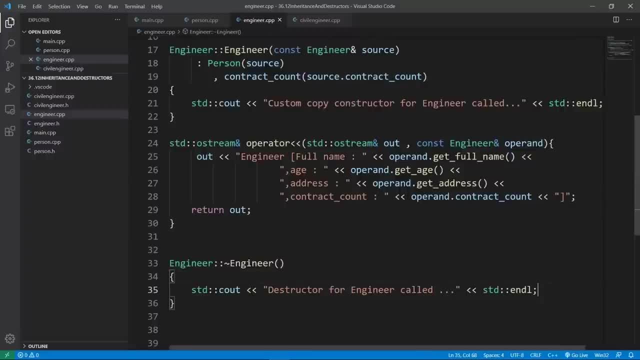 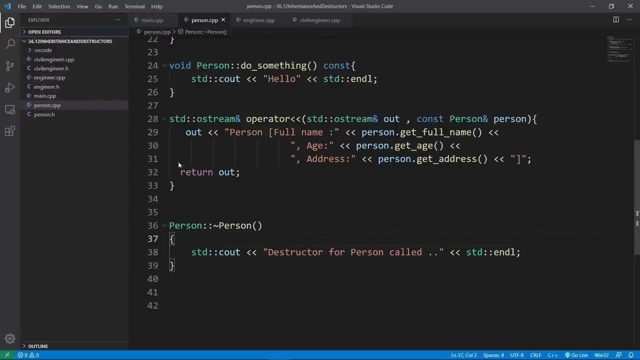 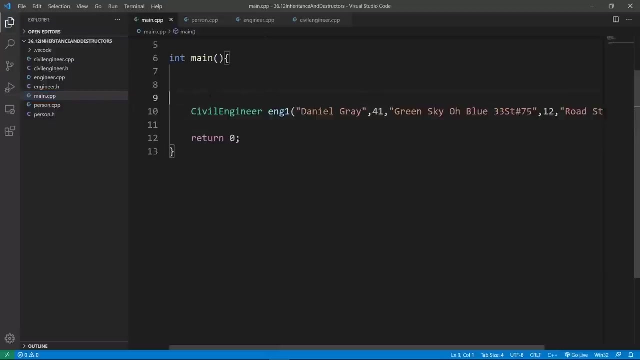 good enough, let's go back and make sure we have the same messages here for engineer and we have a destructor for person called message, and we're going to try and run the code and see how could structures and destructors are called. this is the order we want to make sure we understand. 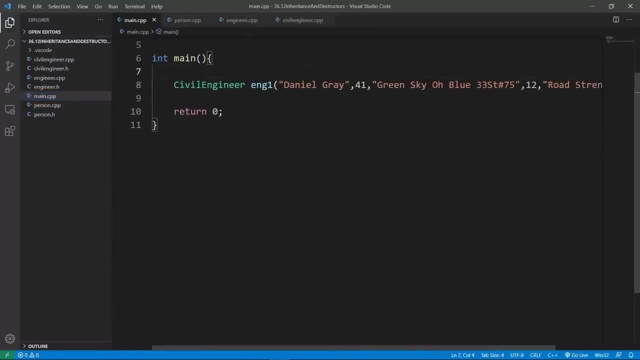 if you want, you can even use a debugger to follow things, but i am not going to do that here. i am just going to build and show you the output statements. hopefully that's going to be proof enough that things happen in the order that i just described in the slides. the build is good, we can. 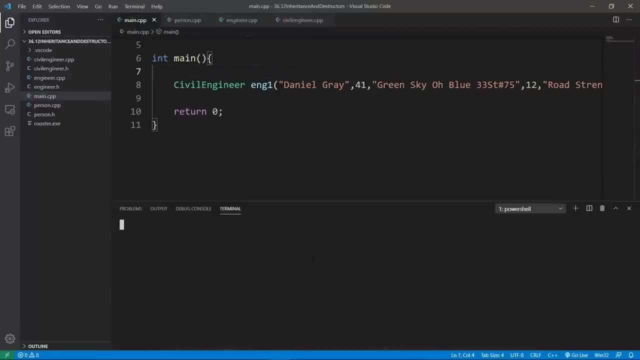 clear. we can bring up a powershell window and then clear and we're going to run rooster, we're going and see the structure will around. and for the constructor stack component, we're going to configure thing about constructors like family year and administrat david like family year and 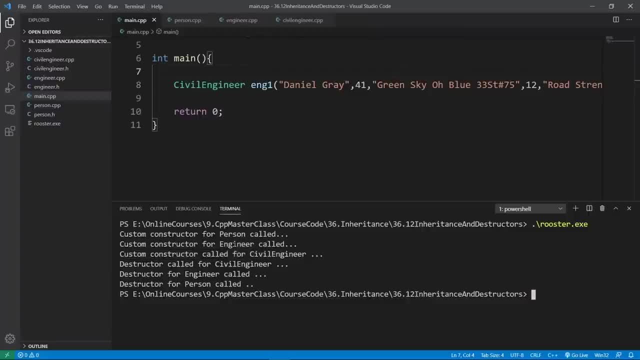 you see that the instructor is going to be called for person for civil engineer, and you're going to see that things are going to happen from the most base constructor to the most specialized constructor. so we are going to call person engineer and civil engineer, but you're going to see that 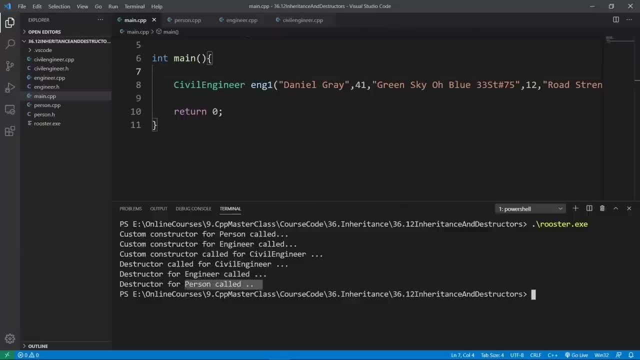 the structures are going to be called in the reverse order for the base class. so things are going to be happening in reverse order. we will build things starting from the base and then finish by the most specialized class which is doing inheritance, and then we're going to call the destructor for the most specialized class first and then. 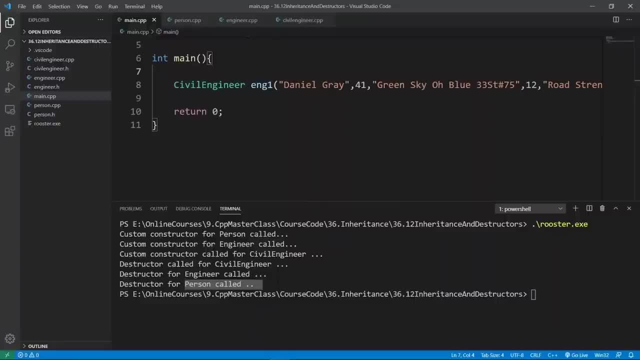 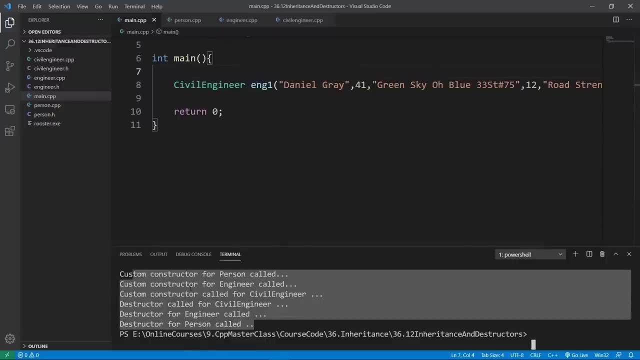 the destructor for the most base class is going to be called last. you should really make sure you understand this, because sometimes your things are going to be depending on this order and you need to understand this and this is really the main message here- that destructors are really called. 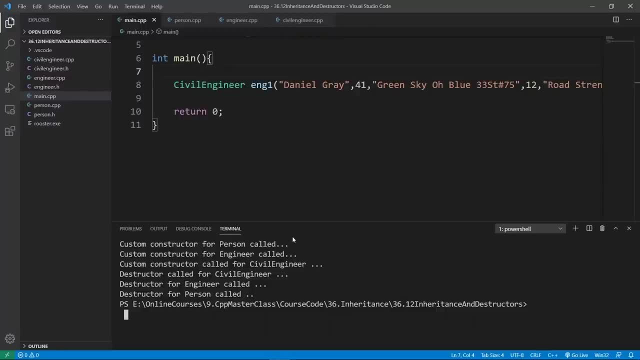 in the reverse order than the constructors. we are going to stop here in this lecture. in the next one we're going to see that we can actually reuse names in our inheritance hierarchy and we're going to see how that works out in the next lecture. so go ahead and finish up here and meet. 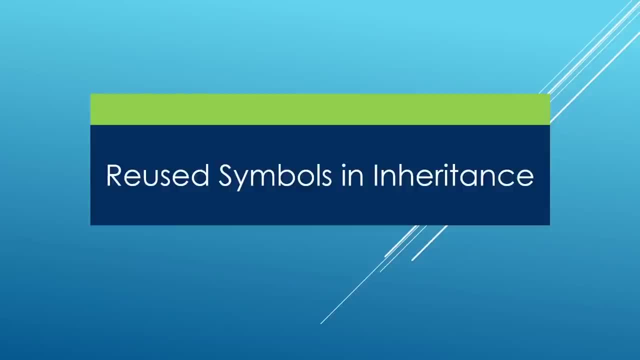 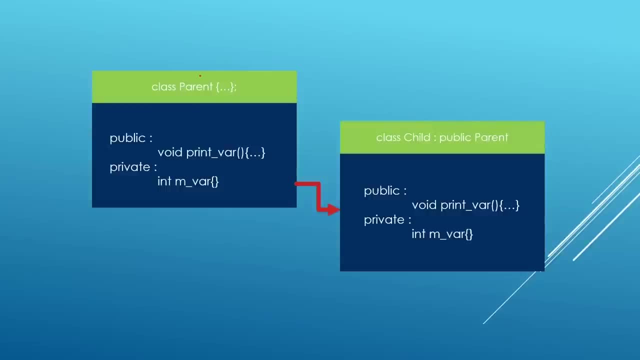 me there in this lecture to see that we can reuse names in our inheritance hierarchy, and what we mean by that is that we can have a parent class, for example, and have a child class inheriting from the parent class and have exactly the same names for the member variables and types or the same signatures for functions. 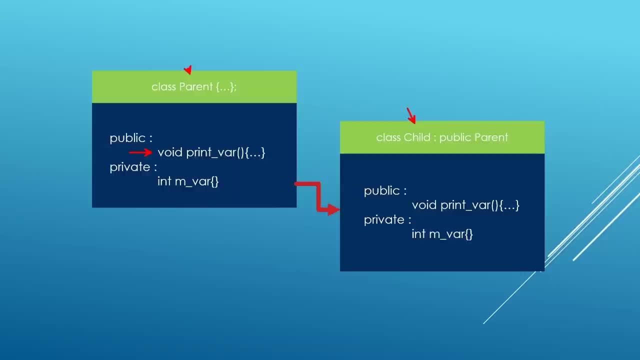 for example, in the parent class, you see that we have a member function called printivore. it is going to be printing some information. we can have a function named exactly the same in the child class and c plus plus is going to allow this. we can also do the same things for member variables. for example, we have m var, which is 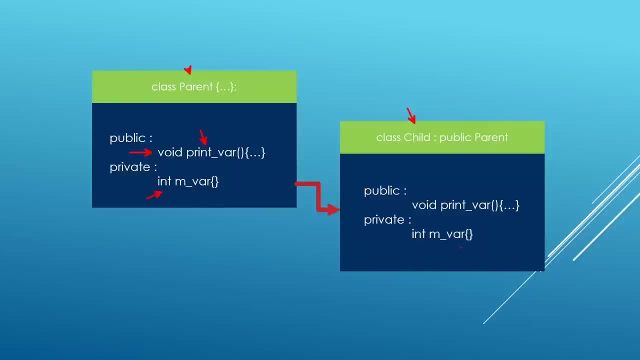 of type and we have exactly the same thing in our child class and c plus plus is going to allow this. now the problem is: if you create an object of child, which method will be called if you call print var. now what c plus plus does is it is going to override or hide things you have in the base class, if you happen to set. 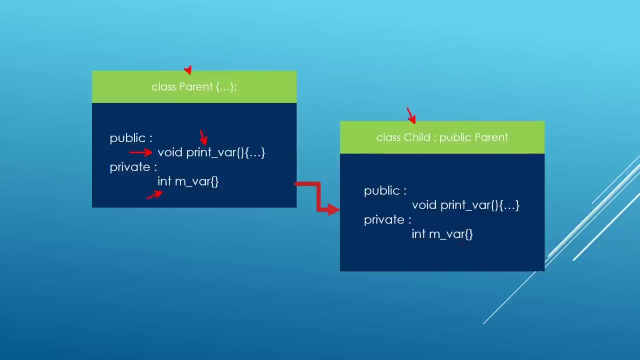 up exactly the same thing in a derived class. so, for example, the members in our child class are going to hide the members we had in the base class and if we call these methods on a child object, we are going to get diversions in the child class code. if we call these methods on a 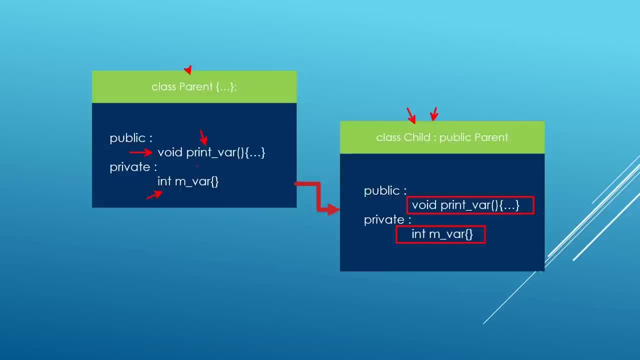 parent object. we are going to get to the parent version called print v, wa and we are going to add lots of separate dog to to the class and if you see that you have that method, i recommend that you see f and e at the same time. now, if you stop the process and we have Longverb which we call print v, 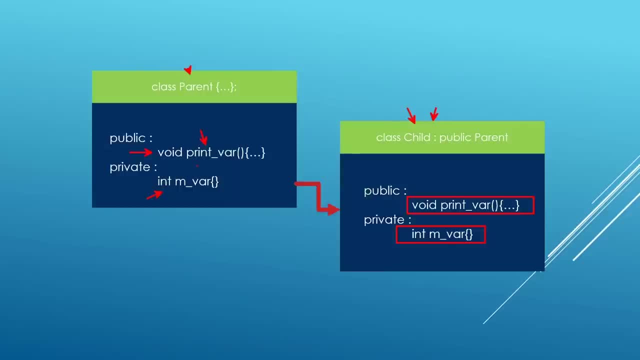 and we're going to see the data in the parent class printed out. this is the message here: it is possible to use the same names in both parent and child classes and if you do that, things in child classes are going to hide or override what we had in the parent class. this. 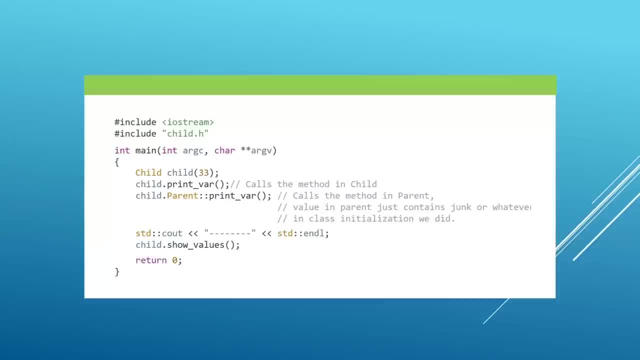 is the message i want to convey here, and here is a simple example to drive home how you can use these things. for example, we can create a child object using this syntax here, and if we call a method on the child object, this is going to call the method in child, but it is possible to force. 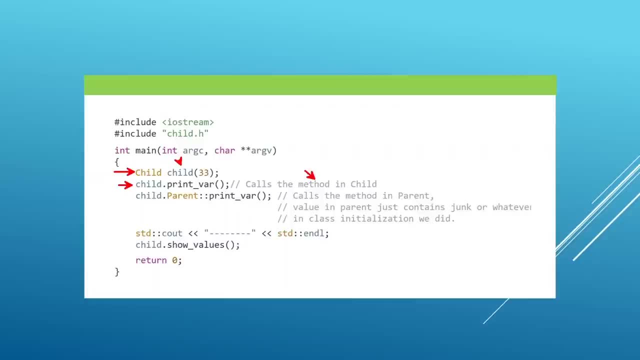 the compiler to call the version in the base class and you're going to see this syntax used somewhere in your code out there. so the syntax is to say the object name. you put it up, you say the name for the parent class and then you call the method using the scope of resolution operator. 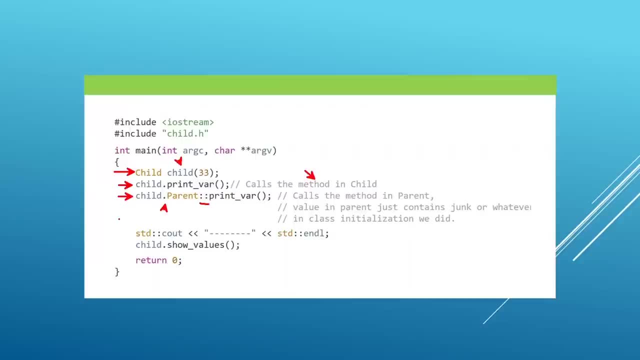 here and this is going to call the method in the parent. okay, now that you know this, we're going to call the method in the parent class and we're going to call the method in the parent class. to head over to visual studio code and play with this a little more: here we are in our working. 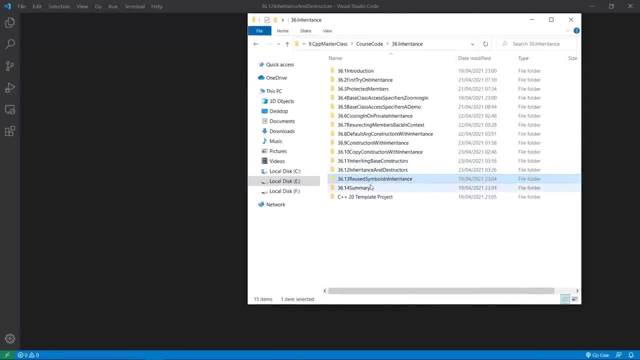 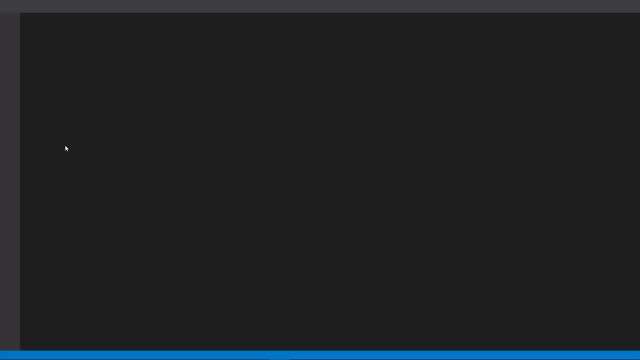 folder the current project is reused. symbols in inheritance. we are going to just grab the template files, because we are going to be building things from scratch here and we're going to put in our files no big deal here and we can open this in visual studio code. this is going to give us. 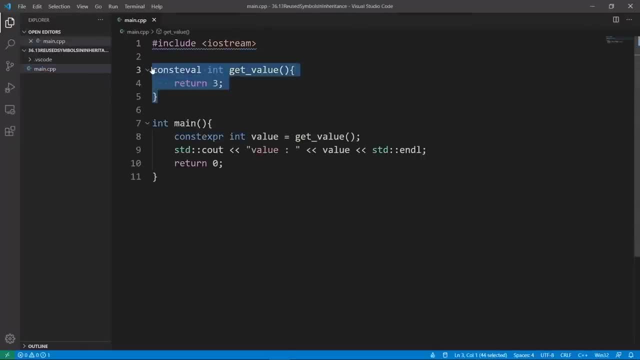 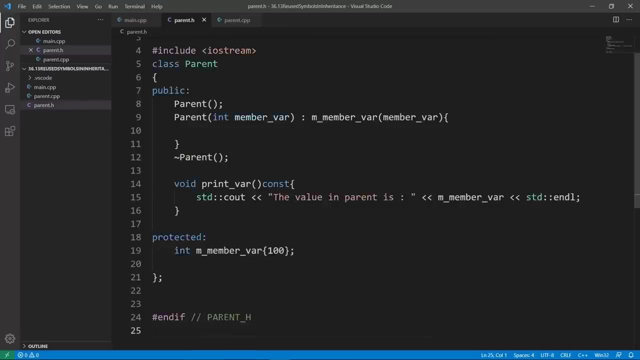 a bare minimum main cpp file. we can clean it up a little bit and we're going to say: setup our parent class. let's do that pretty fast. we're going to say parent and set up the header and we're going to set up the implementation cpp file. we are going to set up the header file and 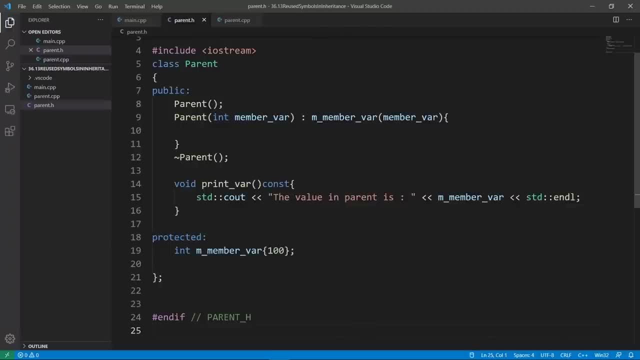 this is going to do everything we want. we have a constructor which is really defaulted here. so let's say default and we can default the destructor. can we default it? let's do this and see what happens, and we don't really need to do anything in the cpp file. we can leave it empty and we can. 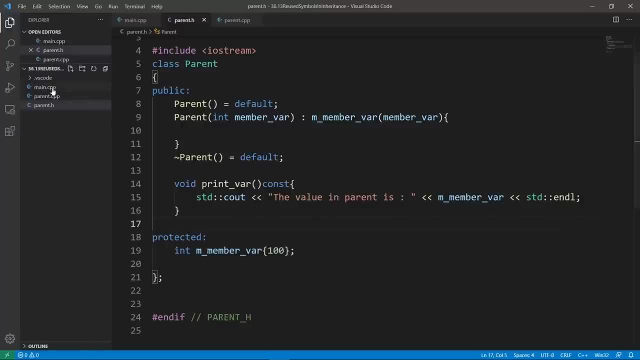 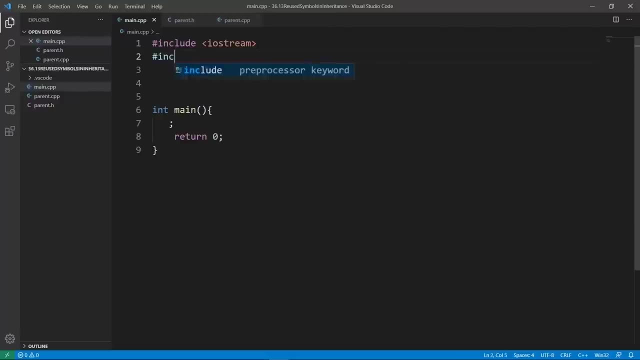 empty. this is not going to hurt anything and with this we can create parent objects. let's do that. we're going to say we're going to hop over to the main cpp file and include parent and make sure that we can use that and we're going to create a parent object. let's do that. we're going to say: 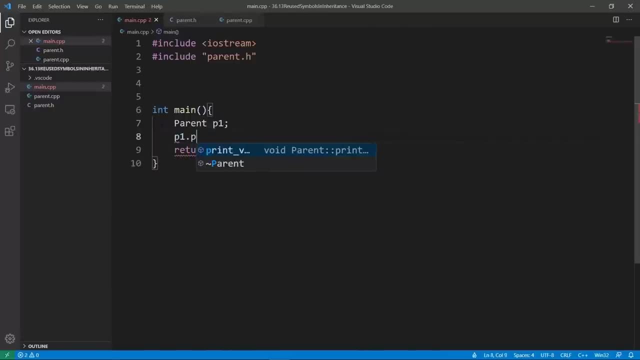 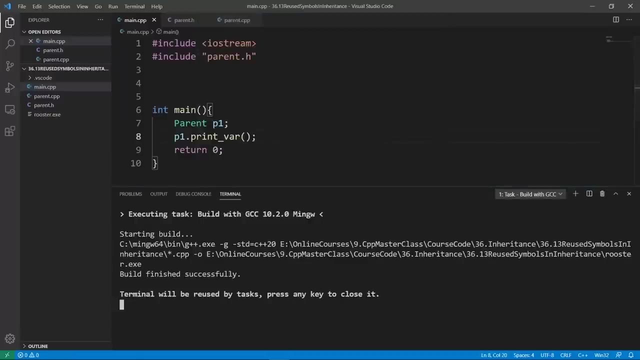 parent p1 and say p1 print values. we can do that and we can build and run this program. i think it is going to work just fine. okay, the build is good. we can clear or we can set up a powershell window and a clear and run rooster. this is going to say: the value in parent is 100, which is what we. 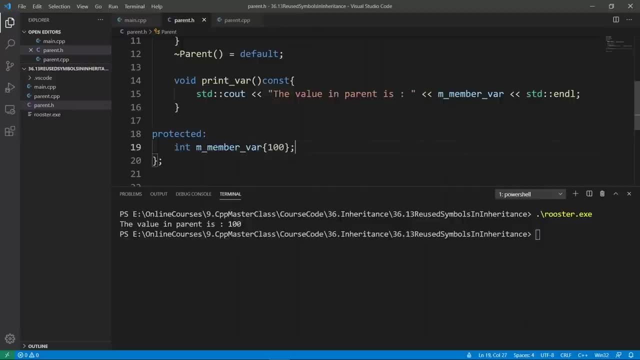 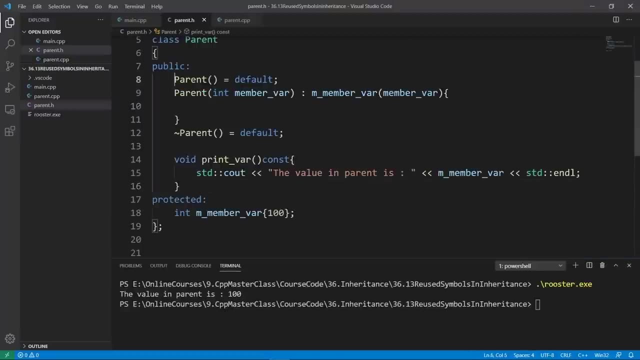 have by default. here we have a simple member variable which is of end type. it is protected because we want it to be inherited. and we have a bunch of constructors here we have a constructor which is going to take a value, but we're not going to use that here. the default is just fine. 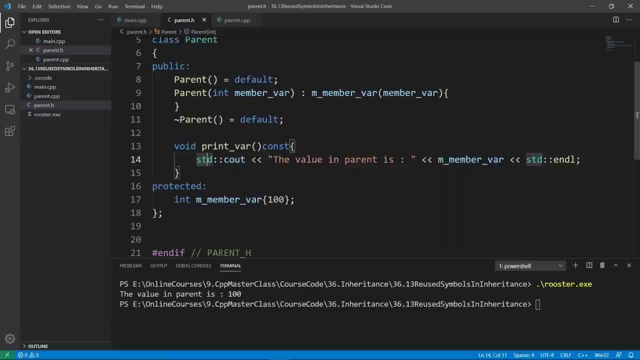 you can use that if you want, and we have a member function which is going to print the value in parent. now that this is working, we can set up a pvc code and we're going to set up the pvc code here. we're going to set up the pvc code and we're going to set up the pvc code and we're going to 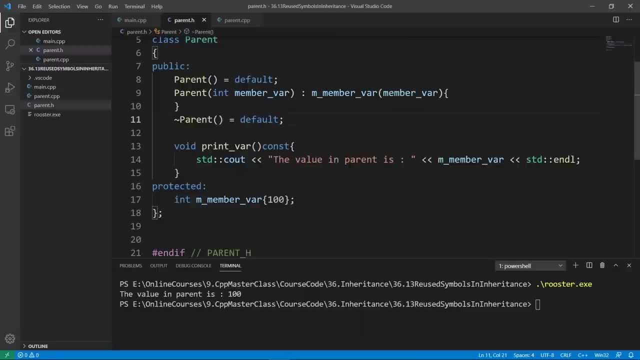 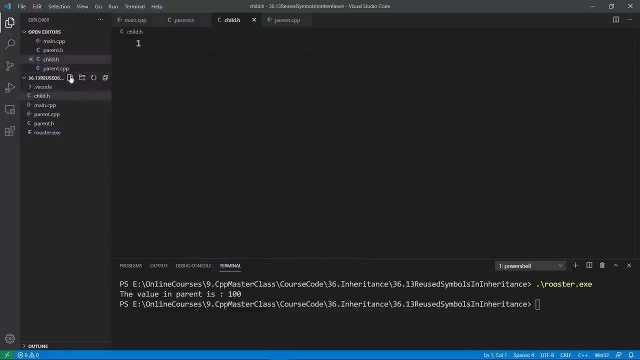 up a child class which is going to be inheriting from the parent class here. so let's do that. we're going to set up the child header file, childh, and we're going to set up a cpp file for that, that cpp. so we are going to put the data in the header file again. it is nothing complicated, it is just. 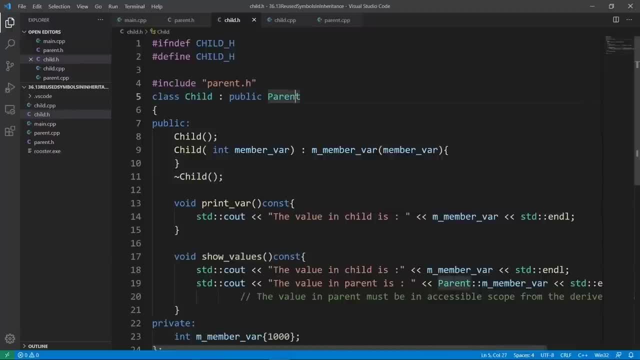 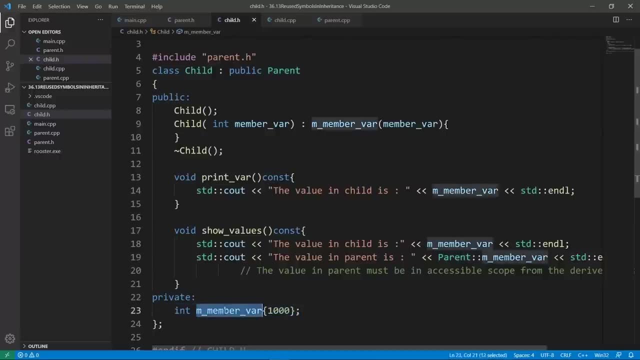 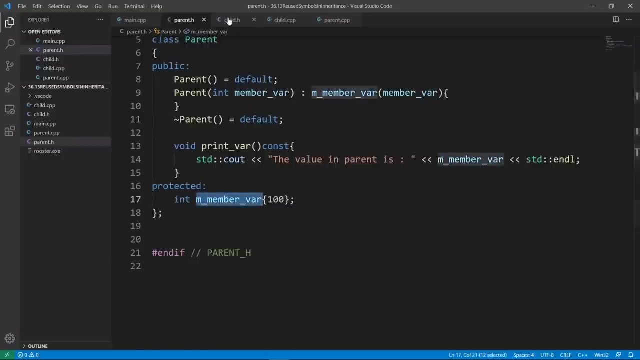 a simple class which is going to be inheriting from parent and we are going to have our own member variable which is going to eclipse what we had in the parent. so the names here must be the same: m member var. if we go in parent, it is m member var and what we have in child is going to 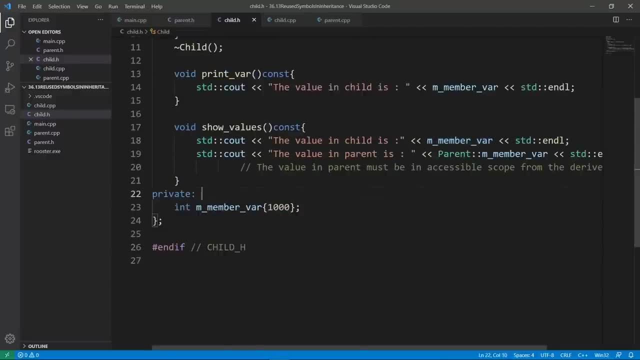 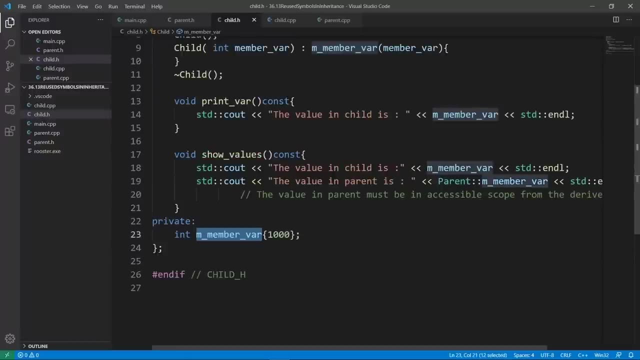 eclipse what we had in the parent class in other worlds. if we print the member variable in child, we're going to see 1000 printed out here. we won't see 100 that we have in the parent printed out. hopefully this is going to drive the point home. 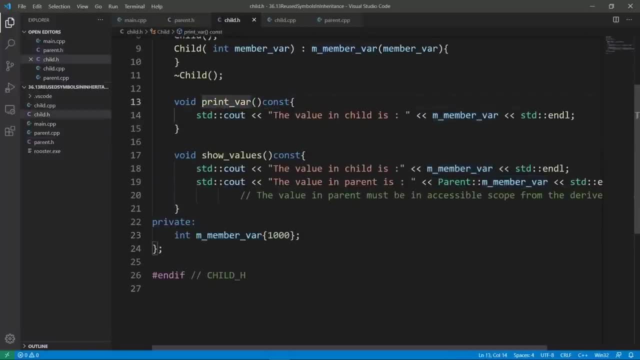 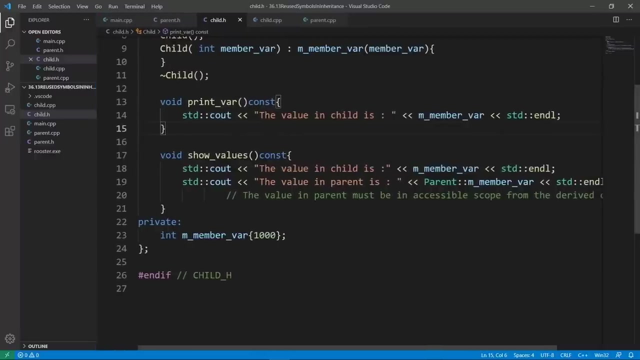 That if you have members named exactly the same, what you have in your derived classes is going to eclipse or hide what we had in the parent class. This is the message here. But even if this is the case, C++ allows us to specify that we want to grab the data in parent from a child object. 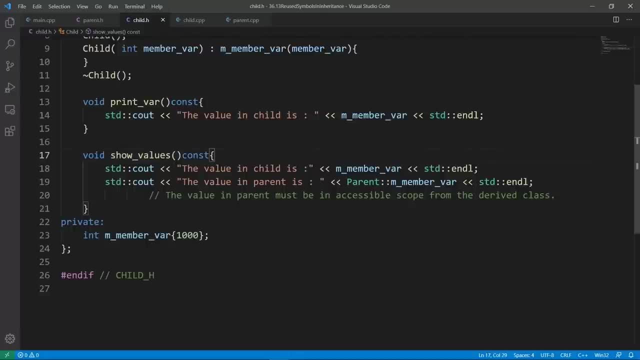 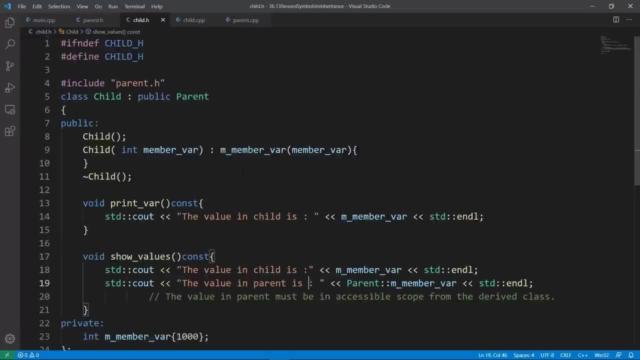 For example, in our show values method we can print the value in child directly using mmember var. But we can also specify that we want the value in the parent class, because even if this is a child object, it has a parent part of it. 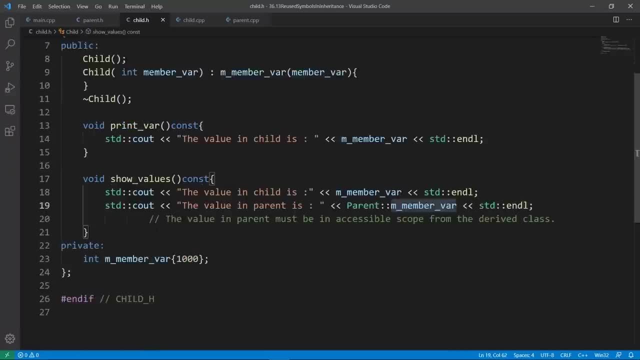 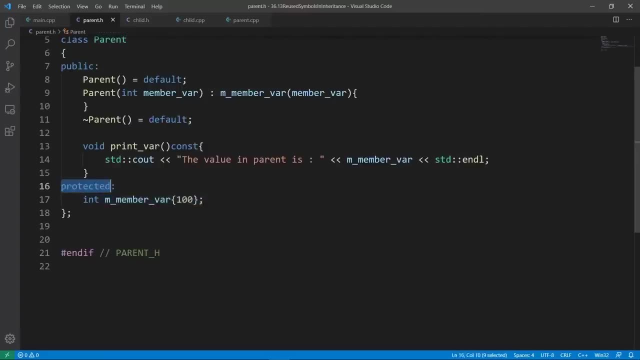 So we can access the data in parent and print that if the data happens to be accessible from our derived class- And that's why we set up our member variable to be protected- for it to be accessible in our derived classes- This is going to allow us to print something like this: 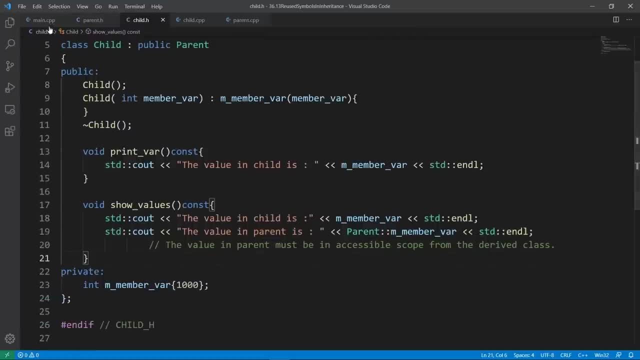 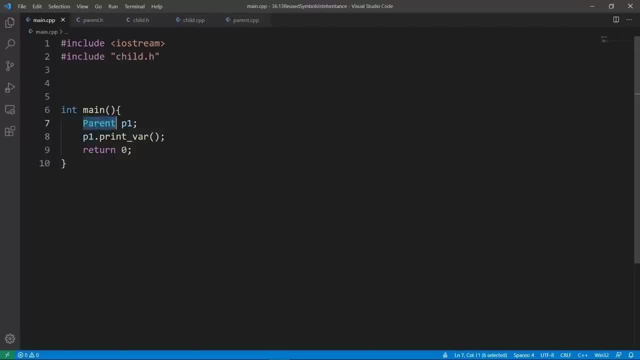 And this is going to really work Now that we have this in parent. We can go in the main CPP file and only include the child. We can do that And we're going to create a child object. Or we can just take out everything here. 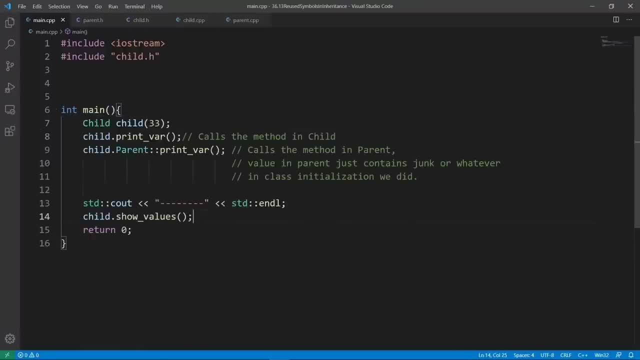 And just put in the code we can use to play with this thing. We can create a child object And on this child we can print var. We're going to see that the data is going to be printed out, But we can also use this syntax to print the data in the parent part of us. 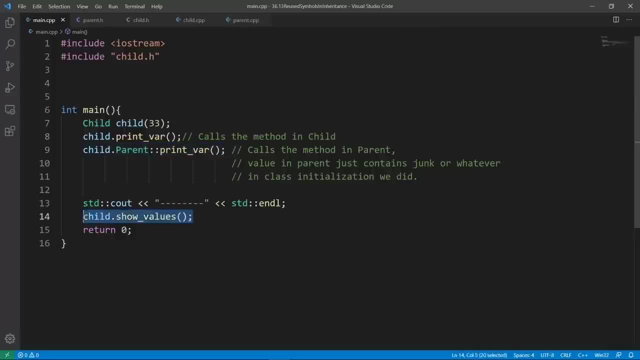 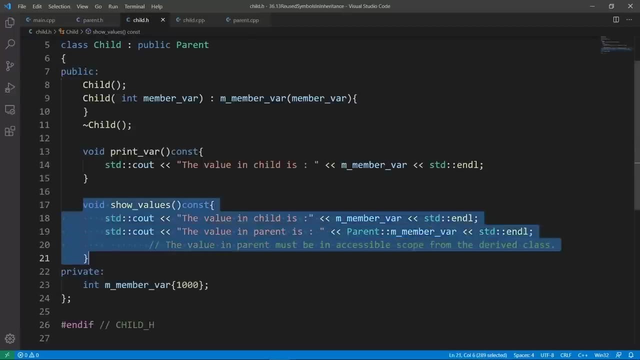 And we're going to see that the data Is printed out. We can also show the values And make sure we see this from a member function of the child class. This is going to call this member And we're going to get the value in child. 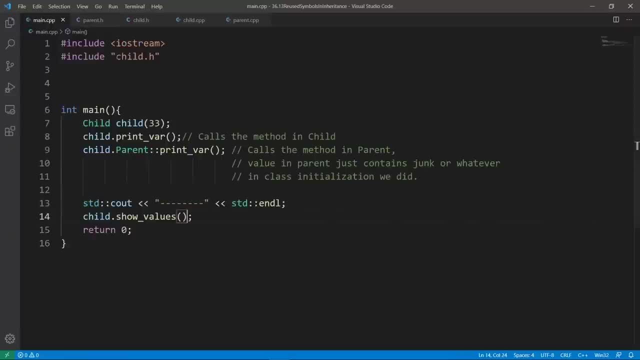 And we're going to get the value in parent printed out on the console. Now that we have this, We can actually try and build this. We're going to use GCC to do that. We're going to see that. we're going to finish building with errors. 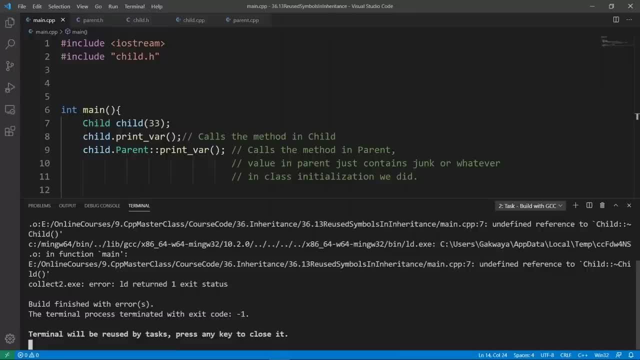 What is the problem here? We have an undefined reference to child Child destructor. We didn't put in a definition for the child destructor, So let's go there And default it. We can do that. We're going to say equals default. 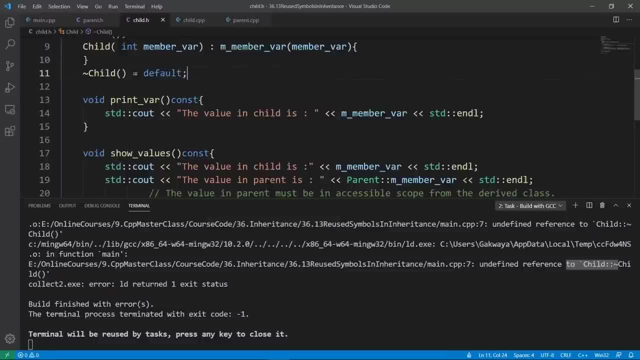 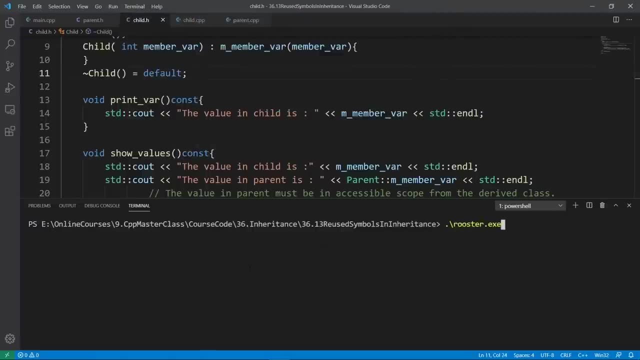 And the compiler is going to generate one for us. And now if we build, We're going to build with GCC again. The build is going to be good. You can clear and run rooster And we're going to see that the value in child is 33.. 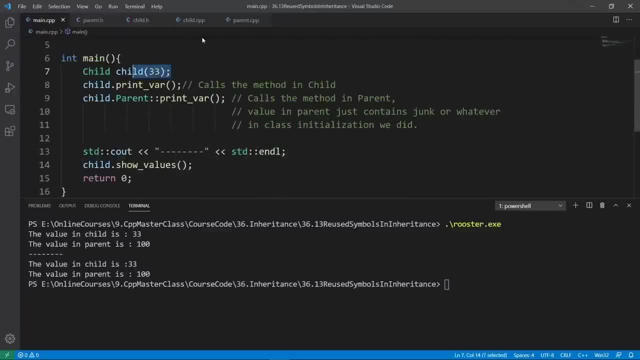 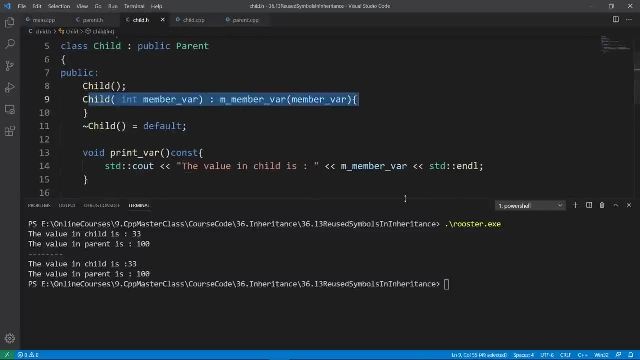 Because we passed that in explicitly And this is going to call The constructor we have in child. That happens to be this guy here. And you see that we are really keeping things simple. We are not calling the base constructor here. The compiler is just going to call. 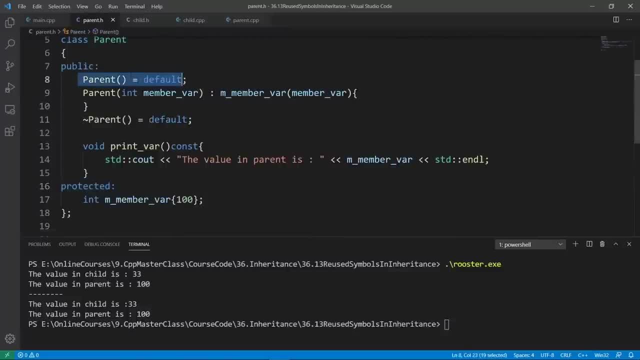 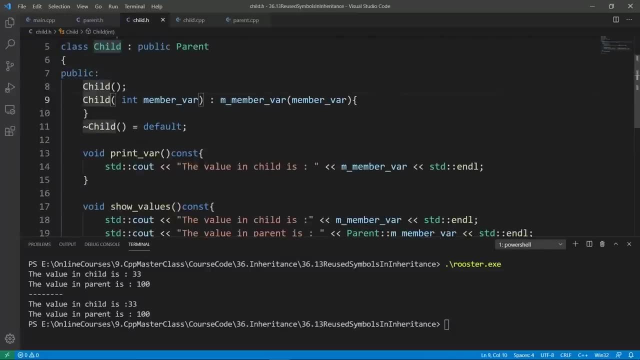 The default constructor we have in parent here And this is going to just work. The main message here is that you can set up member variables And member functions named exactly the same way In the parent class and in child classes And what you have in your. 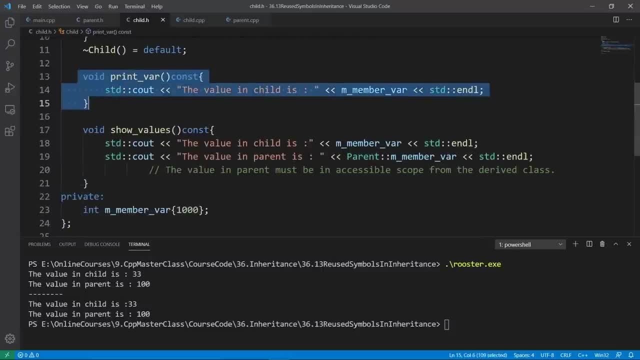 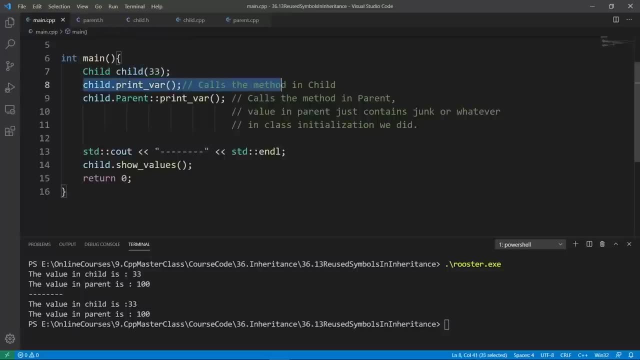 Derived classes is going to hide What we have in our parent classes. So if we call a method on a child object, For example, like we are doing here, This is going to call the method in child, But we still have the ability to call data in the parent part of us. 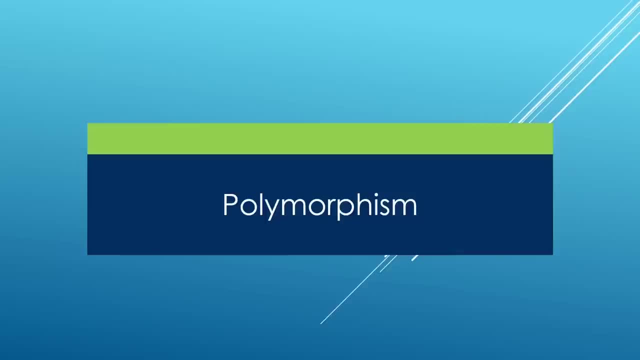 And this is what we do here. I would like to welcome you in this new chapter, Where we're going to be learning about polymorphism, And polymorphism is the setup we can do in our C++ programs To use a base pointer and manage derived objects. 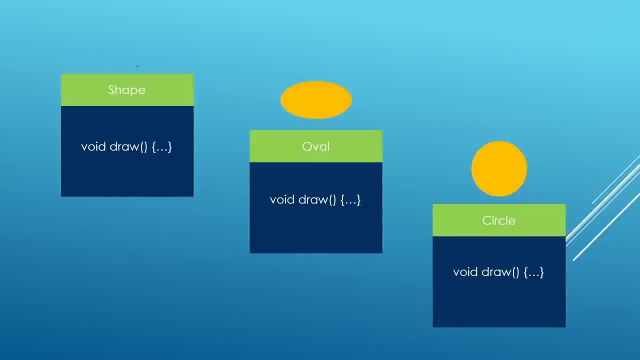 Suppose we have an inheritance hierarchy like we have here. We have shape as our base class And we can inherit from oval and create a circle class. Imagine that we can create all kinds of crazy shapes That inherit from shape in our C++ program. 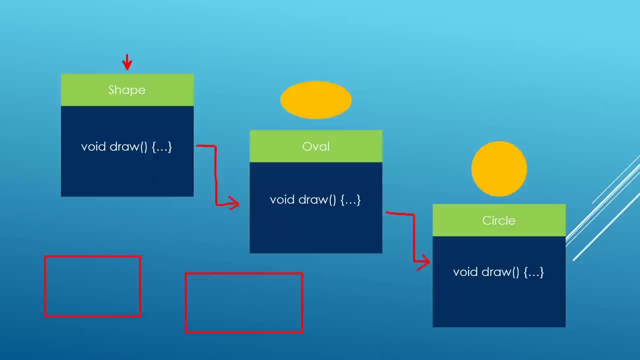 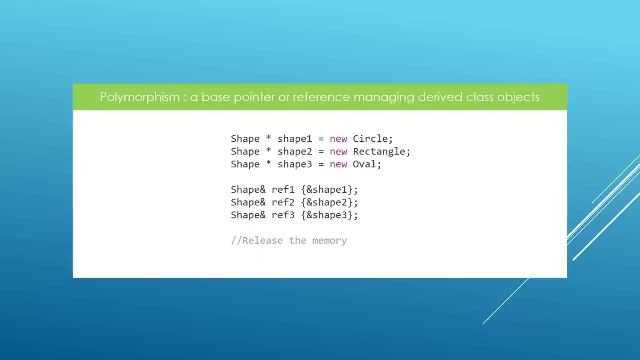 For example, we have a rectangle class, We have a triangle class, We have all kinds of crazy shapes. Now, if we have this inheritance hierarchy, We can create all kinds of crazy shapes. Here is something we might want to do. We might want to set up a base pointer. 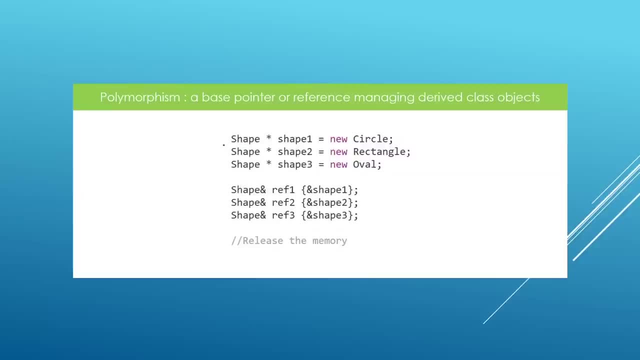 That is managing a derived object, And set up code like this: For example, we say shape pointer And set up a pointer variable here And use this pointer to manage a circle object That we dynamically allocate for on this line. here We can also do a shape pointer that is managing a rectangle. 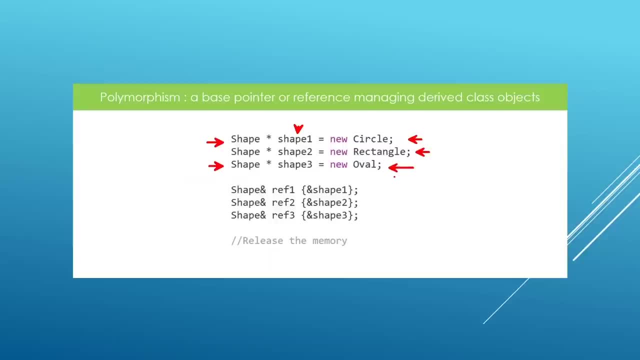 We can set up a shape pointer that is managing a novel object. We can really set up a base pointer That is managing any kind of object we support in our inheritance hierarchy. Now some of you are going to ask a few questions. One of them is going to be: 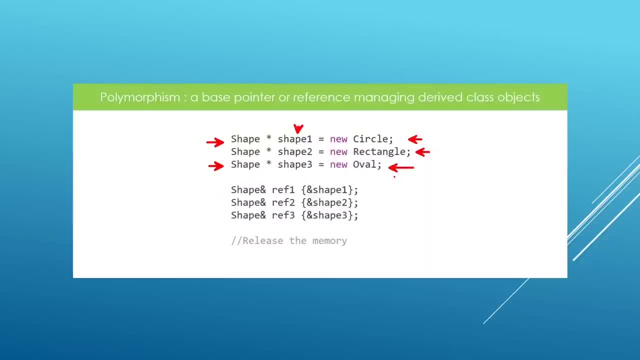 Is this even legal C++ syntax? And the answer is yes, Because if circle is inheriting somehow from shape, A circle is really a shape, And if rectangle is inheriting from shape, It is a shape. And if we try to assign a circle to a shape, 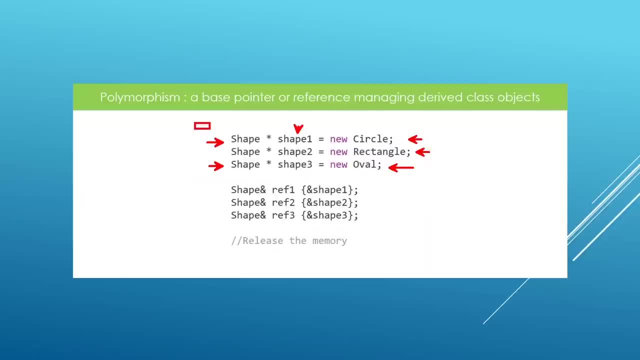 We're going to see that that's going to work. So this is valid C++ And we can do the same thing using references. as we see here. We can set up a reference that is going to be managing a circle object That we have through circle one. 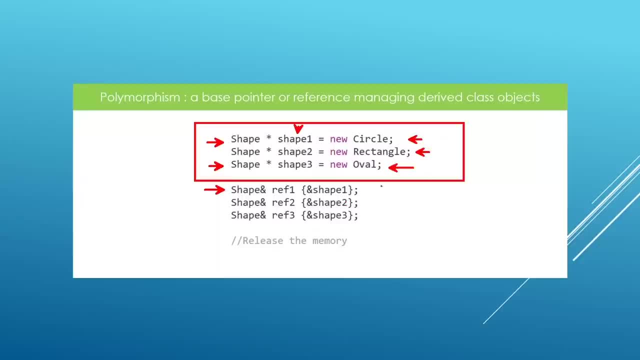 We can set up a reference to manage a rectangle that we have in shape. two, We can set up a reference to manage an awful object. We can really do all these things. Now, some of you are asking: Why would we want to do something like this? 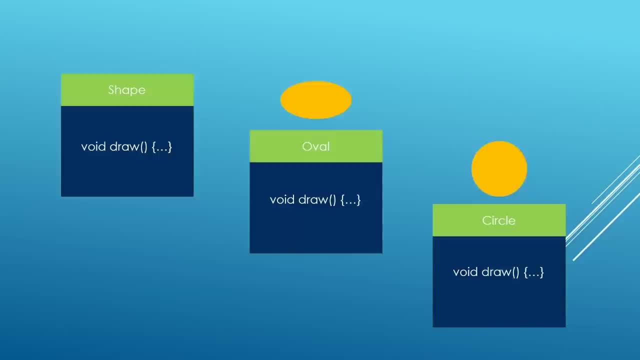 Now try and think about your inheritance hierarchy here And try and think about What if you want to draw this kind of shape. for example, If you didn't use polymorphism, You would need to set up all kinds of crazy methods To draw each kind of object. 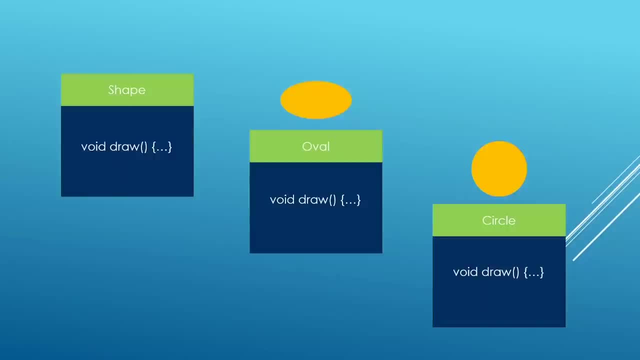 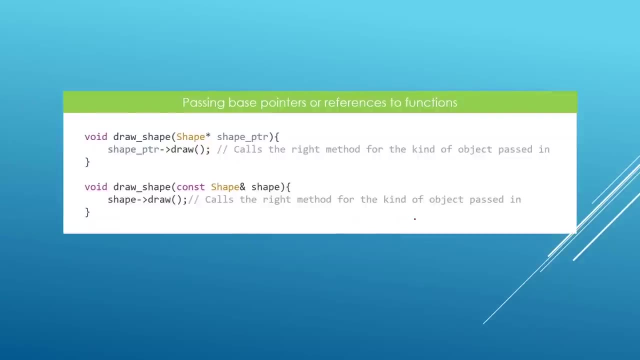 And we have no way around this Because these are different types. If you have a method that takes a novel And you pass in a circle, That's going to give you a compiler error. But with polymorphism We can set up a single method. 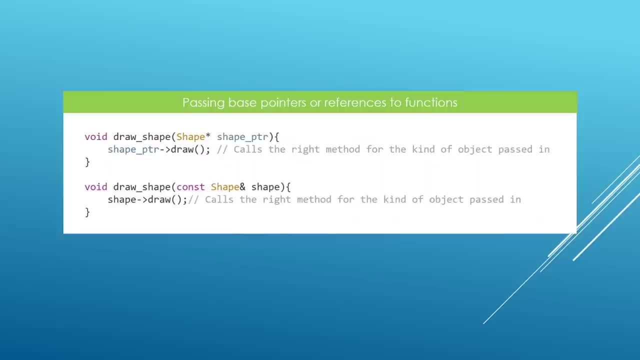 Which takes a shape pointer or a shape reference, And we can pass in All kinds of crazy objects Whose class derived from shape. So, for example, We can pass in the address of the circle And this function is going to draw a circle. 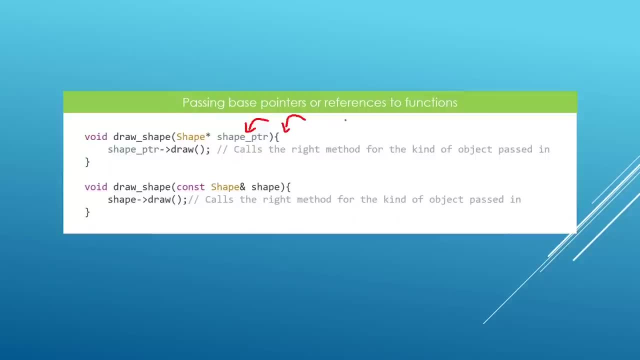 We can pass in the address of a rectangle. This is going to draw a rectangle. We can pass in the address of a novel, And this is going to draw a novel. Hopefully, you can see how this is useful. We can even do this using references. 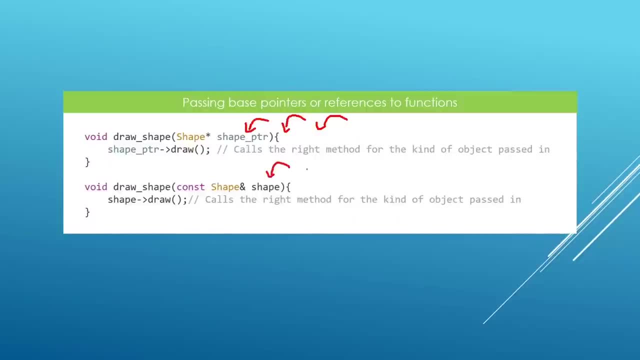 So if we pass in a rectangle, This is going to draw a rectangle. If we pass in a circle, This is going to draw a circle. You get the idea. This is one Of the benefits of using polymorphism. Again, polymorphism is about 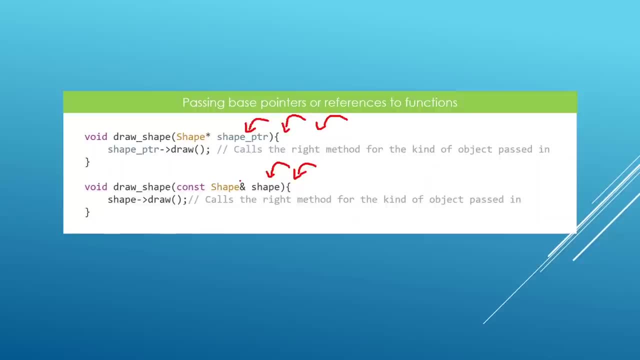 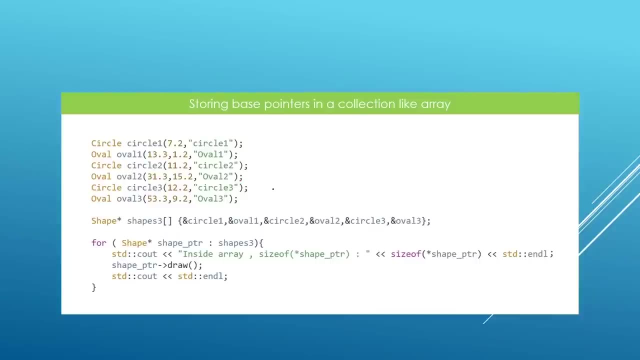 Using base class pointers or references To manage derived objects In our inheritance hierarchies. Another benefit of polymorphism Is to allow us to be able to store Different kinds of objects In a single collection. Remember, an array can't store. 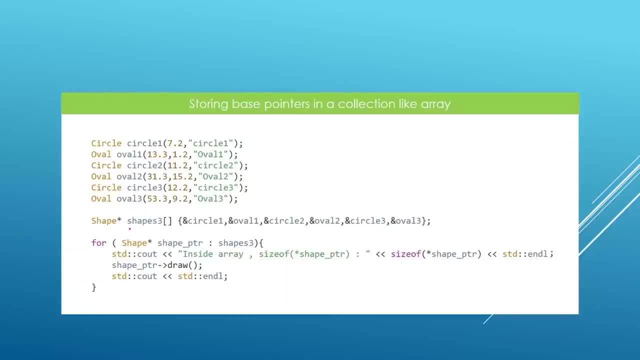 Objects of different types. If you set up an int array And try to store in a string or a double, You're going to get a compiler error Because that's not allowed. So if you have an array That is going to store circles, 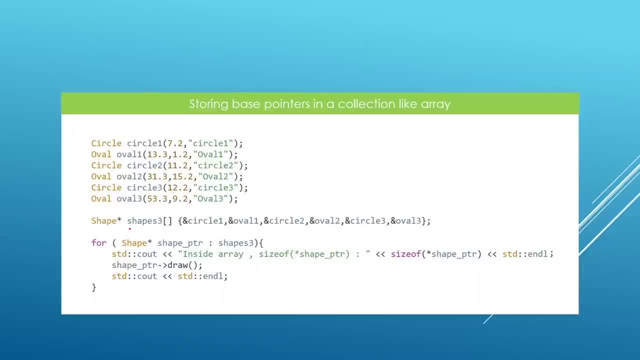 You can't put in a novel, You can't put in a rectangle, You can't put in a star, You can't really do that Because an array, by design, Is going to store objects of the same type. But we can avoid this limitation. 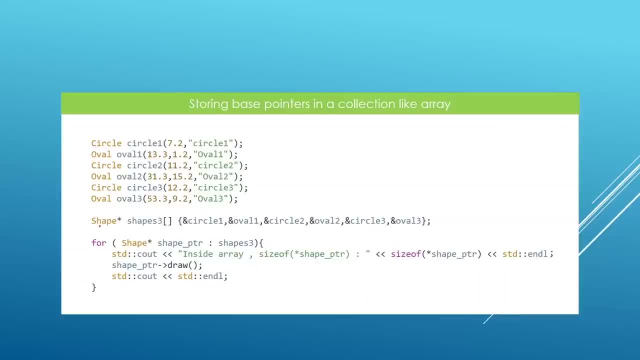 Using polymorphism Again, we can set up an array That is going to store base class pointers And we can store in All kinds of crazy objects Whose class derived from This base class here. So here we can store in a circle object. 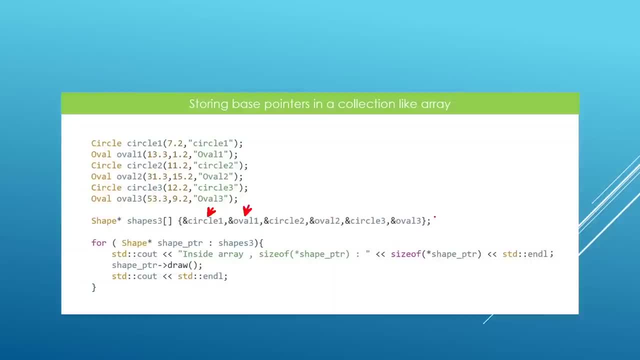 We can store in a novel, We can store in any kind of object That is part of our inheritance hierarchy, With the base class as shape, And this is going to work And this is going to be using polymorphism, For example, if you look through this collection, 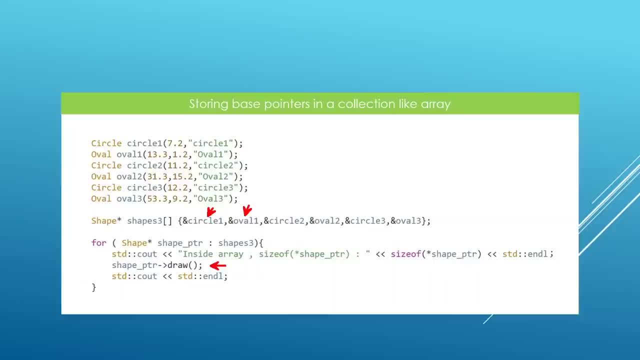 Calling the draw method. For the first element, This is going to call the draw method on the circle. For the second element, We're going to call the draw method on a novel, And this is going to be really cool. This is something. 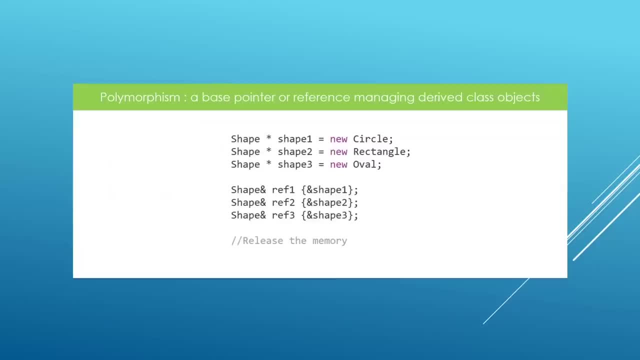 We can achieve with polymorphism, And I want to back up a little bit And talk about what is really meant by polymorphism. Polymorphism really means multiple forms And, in my opinion, What this means is that The base class pointer. 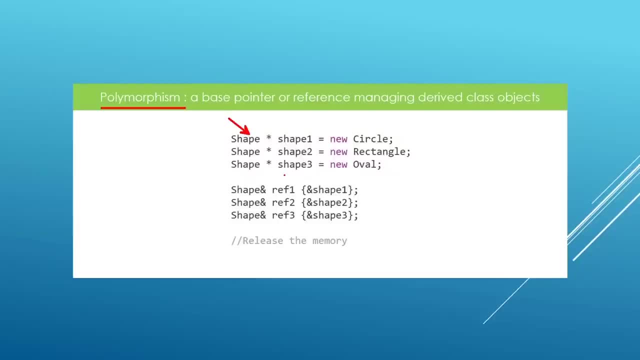 Or base class reference, Can take multiple forms: At one point it might be managing a circle, At one point it might be managing a rectangle, At one point it might be managing a novel object. So it is a base pointer, But it can take multiple forms. 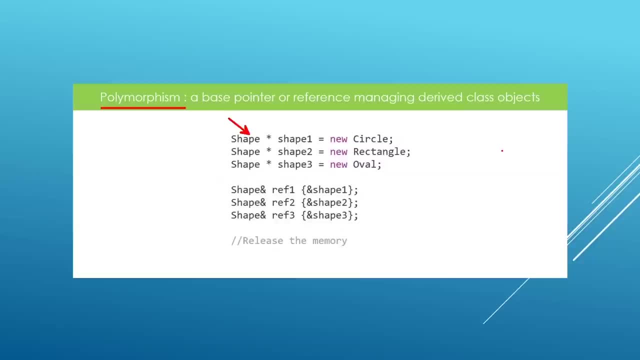 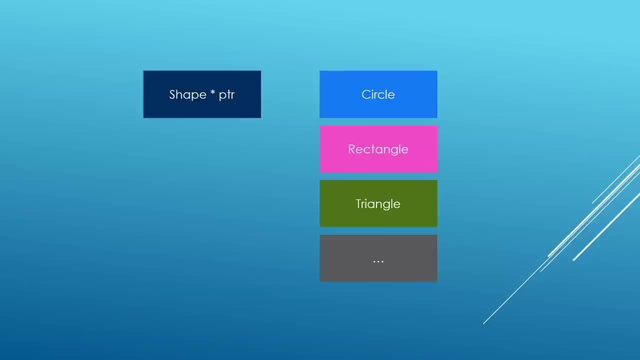 Because it can be managing multiple kinds of objects Whose class are part of our inheritance hierarchy. This is what we mean by polymorphism. So again, the idea is that We can use a base class pointer Or reference to manage all kinds of crazy objects. 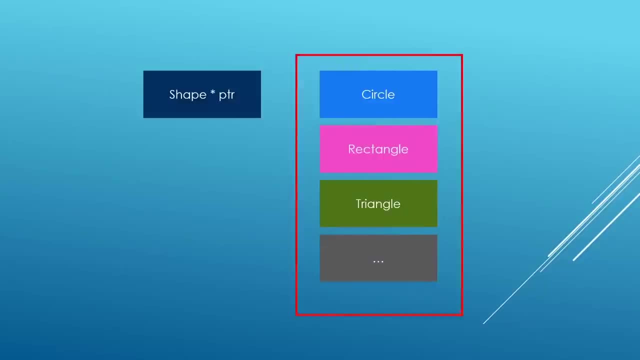 In our program And this is going to have many benefits, As we are about to experience In this chapter here. I am really excited to be explaining this to you. This is one of the most powerful features in C++. We are going to start. 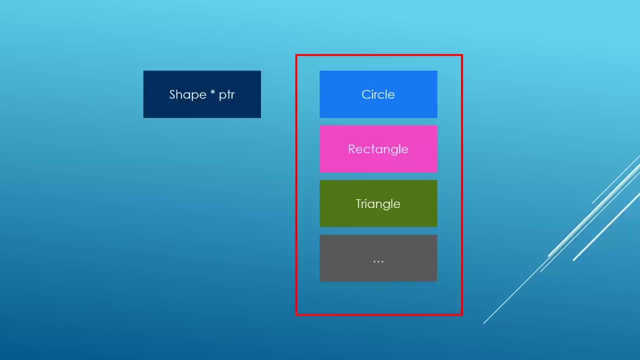 In the next lecture And show you that you don't get polymorphism By default in C++ And what you get is static binding. Go ahead and finish up here And meet me there: Manage derived objects in our C++ program. Hopefully this is going to give you. 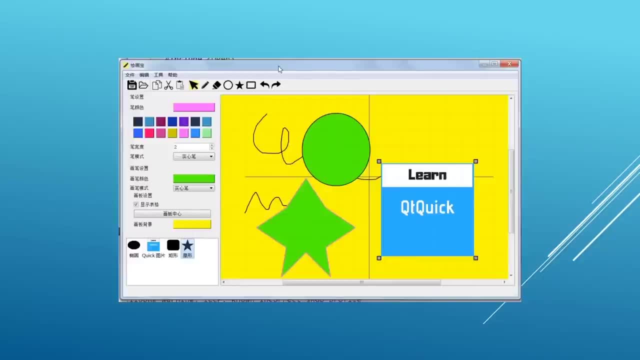 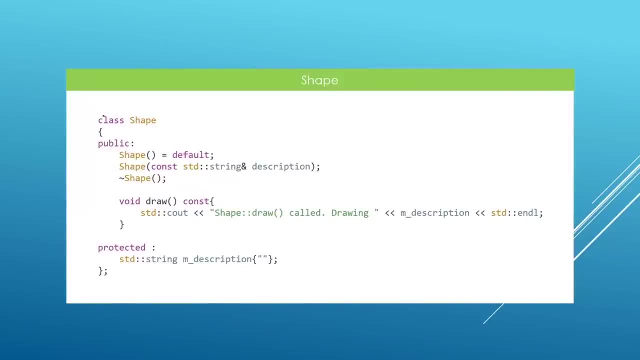 A clear idea On why we might need to do this. So let's look at our classes That we are going to be using here. We are going to set up a shape class, Which is going to be representing our shapes. This is going to be our base class. 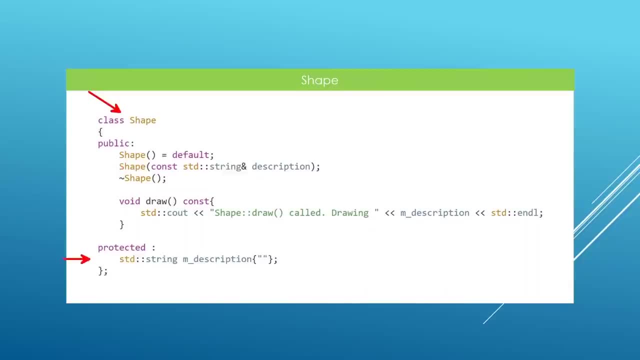 That's the basic use for this. here It has a simple member variable Which is going to store the description For our shape. It is also going to have our draw method, Which is really not going to draw anything. It is just going to say the description. 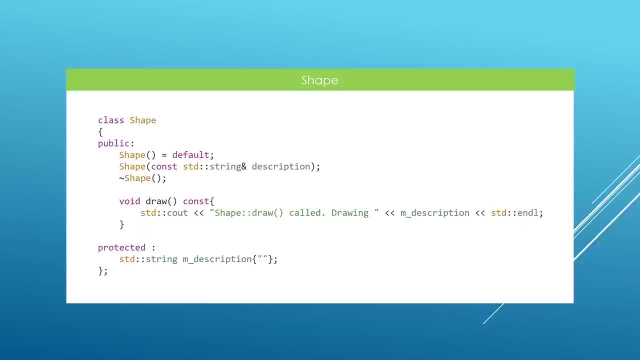 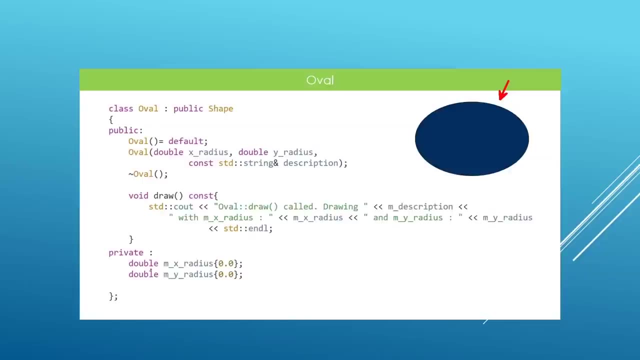 For our shape here. Once we have this shape, We can create other shapes from it. For example, we can create a novel class Which is going to be representing a shape like this. It is going to have two member variables. One is going to be MX radius. 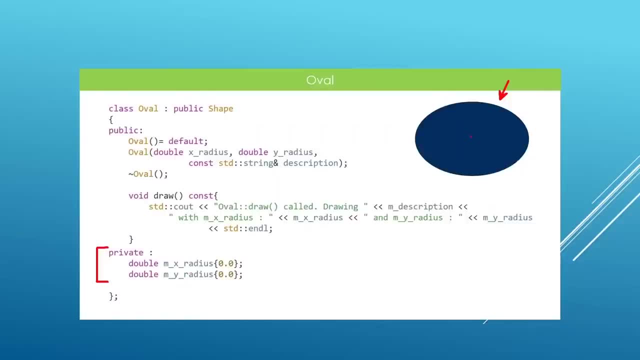 the other is going to be my radius. this may represent the radiuses for our oval here, for example, the x radius might be something like this, the y radius might be something like this, and this is how we're going to be representing this shape. here we also have a draw method which is going to 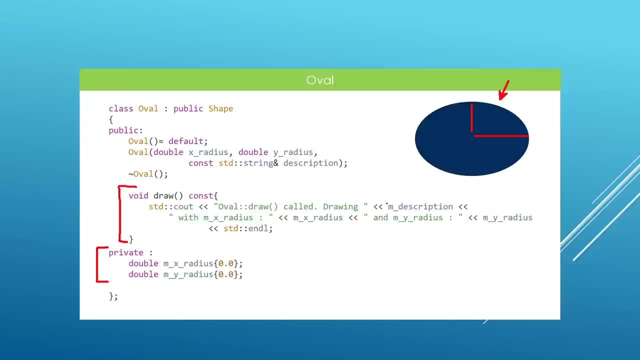 print the information about this shape here. it is going to say the description that we're going to be inheriting publicly from shape, but it is also going to say the radius information for this shape. it is going to give us the x radius and the y radius here, and we have a bunch of constructors. 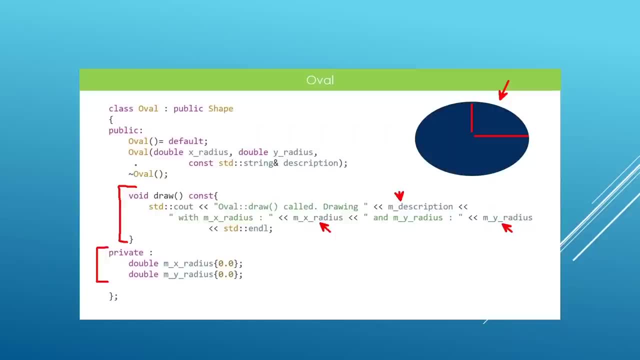 here we have a default constructor, which is really not going to do anything. we also have a constructor that is going to be taking two parameters to forward the data in our member variables here. this is the kind of class we're going to set up in our program. we also have another. 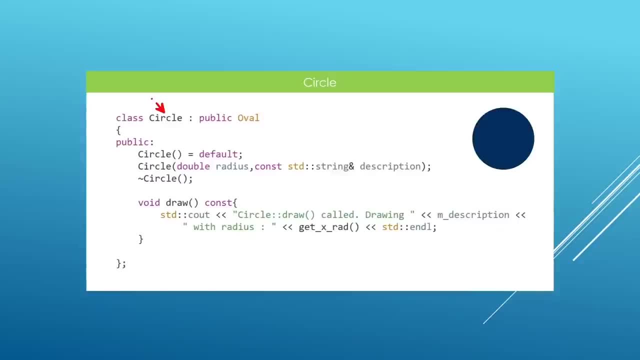 derived class from oval and this is going to be a circle class. it is going to be a specialization on oval in which both x and y radius are equal. so the x radius is going to be something like this and the y radius is going to be something like this, and both of these are going to be equal. so this is going to 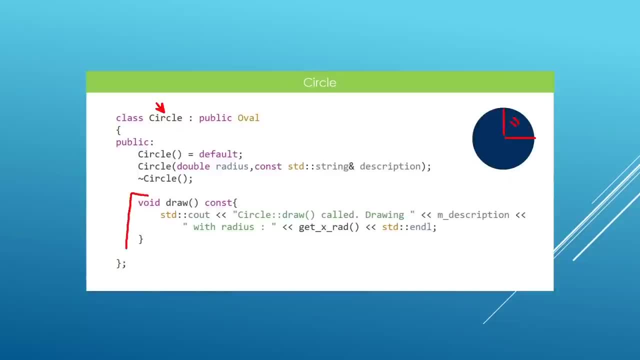 give us a circle shape. we also have a draw method which is going to print the description and the radius. we can really pick any radius. we can pick the x radius, we can pick the y radius. they are really going to be the same because they are equal for our circle shape. we also have a simple constructor which is going to take the 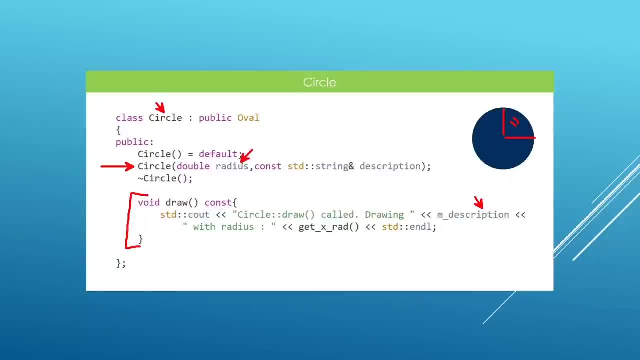 radius, and we are going to be using this radius to forward the data to our oval part of us, and we're going to be setting this as both x and y radius. this is the setup we have here. okay, now that we have our inheritance hierarchy, we're going to try and use it and 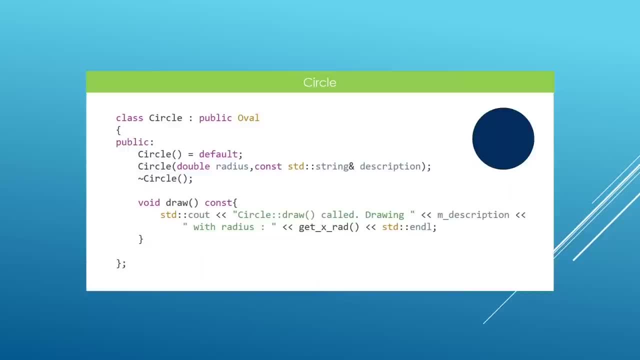 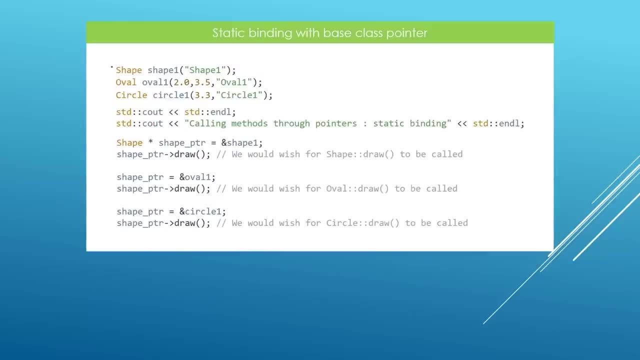 really explore the idea of static binding in c++ inheritance hierarchies. so here we are trying to create simple objects of our classes. we have a shape object, we have an oval object and we have a circle object. we are going to go through a base pointer and try to manage our objects here. 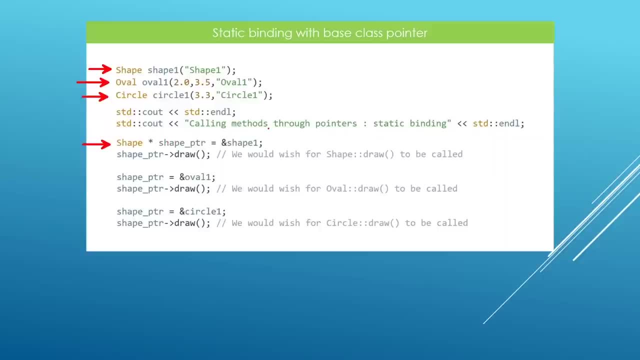 in our first line. we're going to set up a shape pointer and we're going to store in the address of shape one and what we would want you know c++ program is that if we call the draw method on this shape pointer, we would want the shape draw. 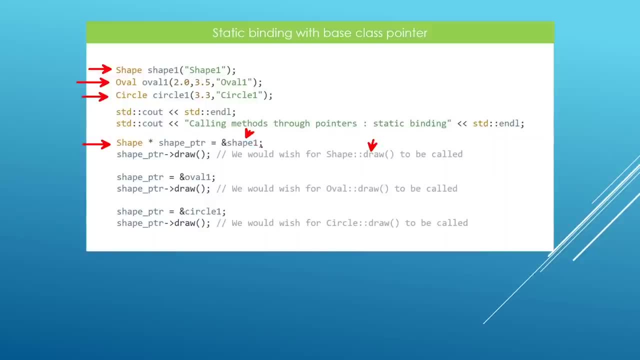 method to be called. because we have a shape object stored in our base pointer here or in other worlds, we are using a base pointer to manage this object in memory down. here we store an awful object in our shape pointer, or in other words, we're going to be using this base pointer to manage an actual 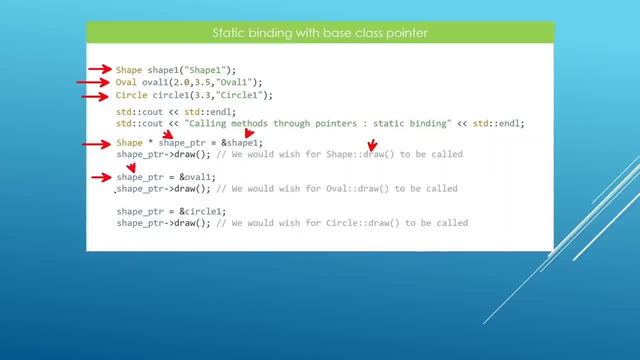 oval object in memory. so we will be doing that here and we're going to set up this space pointer as a in memory. and the setup we want is that if we call the draw method on this shape pointer now, we are going to get the awful draw method to be called. this is: 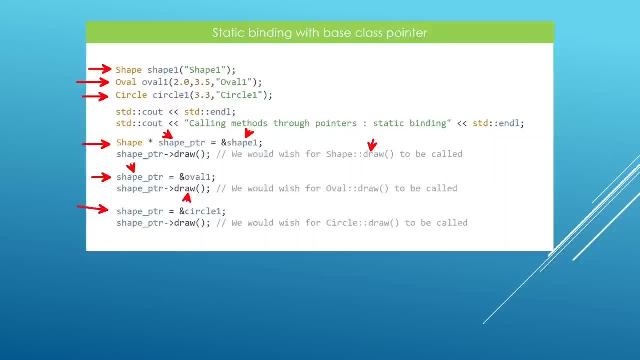 the setup we want. and down here we have another example where we are using this base pointer to manage a circle object. we are going to store the address of the circle object in this base pointer. this is how we do this, and when we call a draw method on this base pointer, we want the circle draw method to be called. so 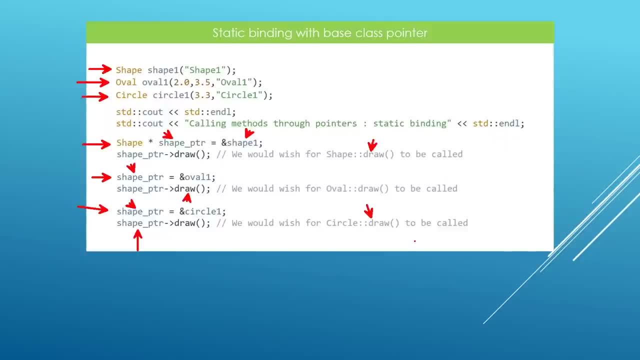 with polymorphism. what we really want is to call a method on the base pointer and get the most specific possible method called on our pointer. this is the setup we want, but this is not what we get by default in C++. if you happen to do this, 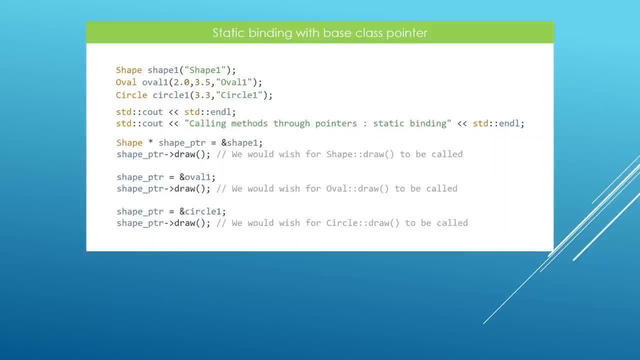 and run our program as is now with the current knowledge that we have. on the first line here we're going to get the shape draw method called. this is what we want. but on the second example here we will see that we see the shape draw method also called, and on this line we will also see that we get the shape. 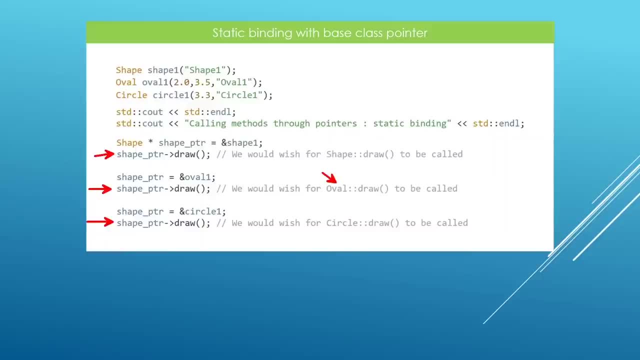 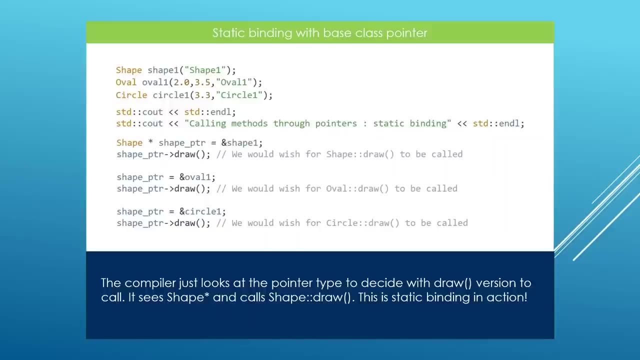 draw method to be called. this is not what we want and this is static binding. so what is happening here is the compiler is looking at the type of the pointer and it is using that to decide which draw method to call. so the compiler is right. so the compiler is basically saying: I have a shape pointer. 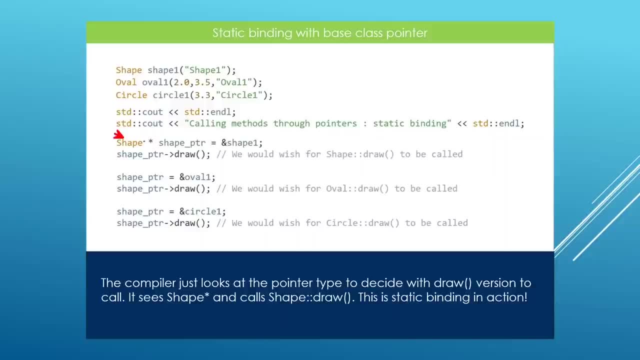 so I am going to call the draw method on the shape class. down here it is going to see that it also has a shape pointer. and it is going to call the draw method on shape, and down here it is going to see that it has a shape pointer and it is. 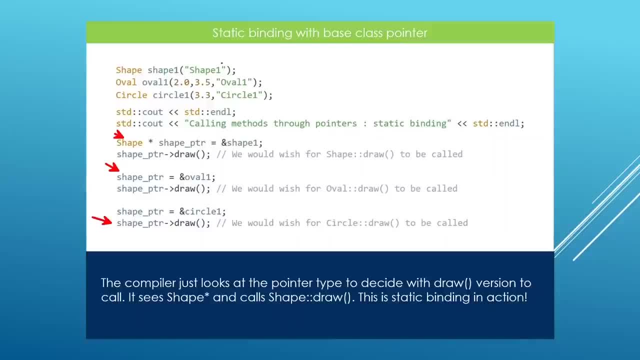 going to call the draw method on the shape class. this is what static binding is all about. the compiler is going to resolve the draw method statically, and what that means is that the compiler is going to look at the type of the pointer that we have and it is going to use that to decide which draw method to call in. 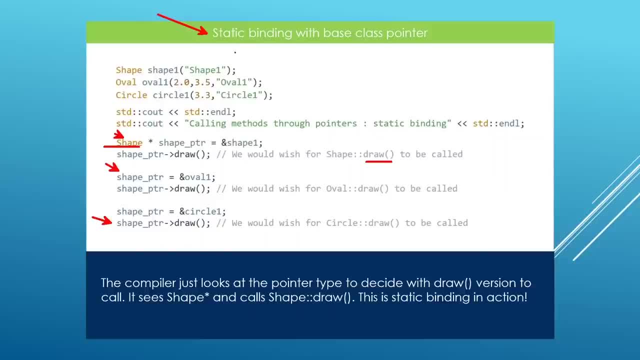 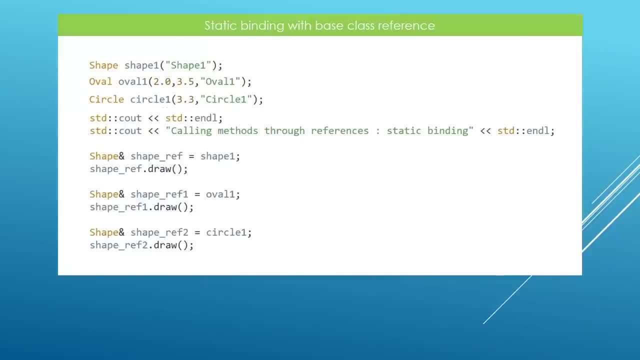 our inheritance hierarchy. so this is the default and it is called static binding. in C++ we also get to the same behavior if we try to use a base reference to manage our actual object in memory. here we have the same kinds of objects we had in a previous slide and we are using a base. 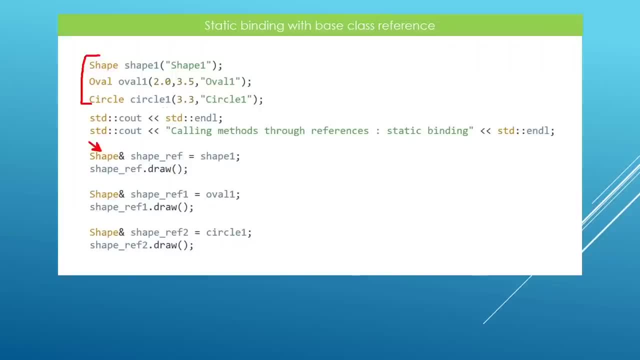 reference to manage our object. and what we really want is that if we go through a base reference to call our draw method, we will get the most specific draw method called. so if our base reference is managing a shape, we will get the shape draw method called. if our base reference is managing another object, we 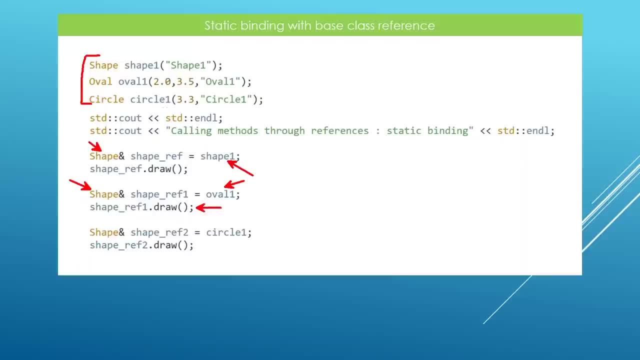 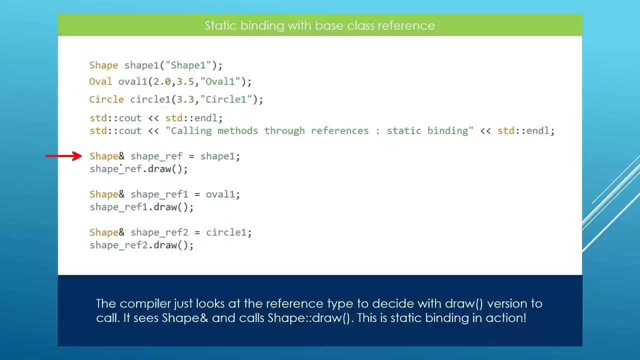 want the awful draw method to be called here, and if our base reference is managing a circle object, we want the circle draw method called here. this is what we want. but again, the compiler is just going to look at the type of the reference. so for the first line here it's going to say: I have a shape reference, so I am going to call. 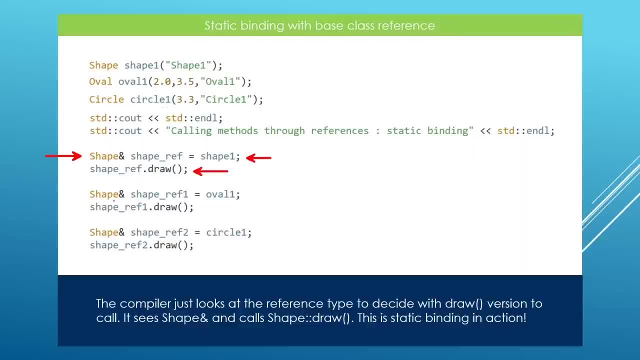 the shape draw method. that's what we're going to get here. on the second line: here it's going to say: uh-huh, I have a shape reference, so I will call the draw method of the shape class. that's what we're going to see here by default. and on 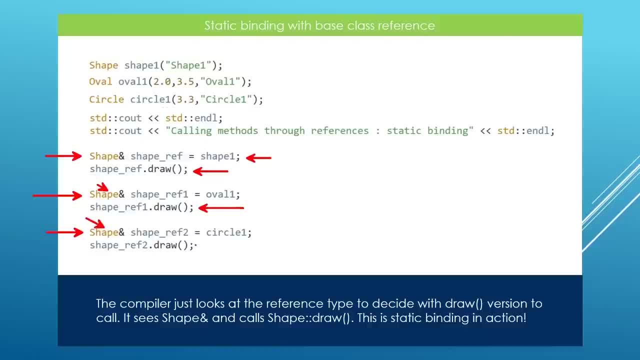 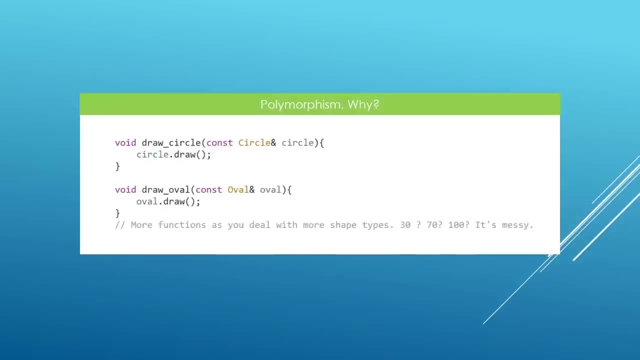 this line here. it is going to say: I have a shape reference, so I am going to call the draw method on the shape class and this is the behavior we get by default and this is static binding in action. okay, so now that we have seen what static binding is all about, let's re-examine the idea of why we need. 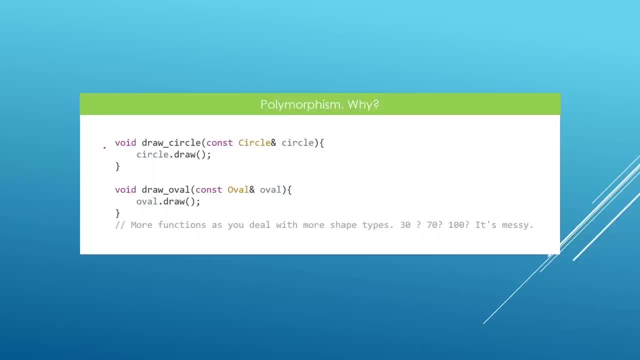 polymorphism, and I am going to give you a simple example here. suppose we have a bunch of shapes we manage in our program and we have a bunch of shapes that are in our programs and we want to draw all these shapes. if we want to draw a circle, 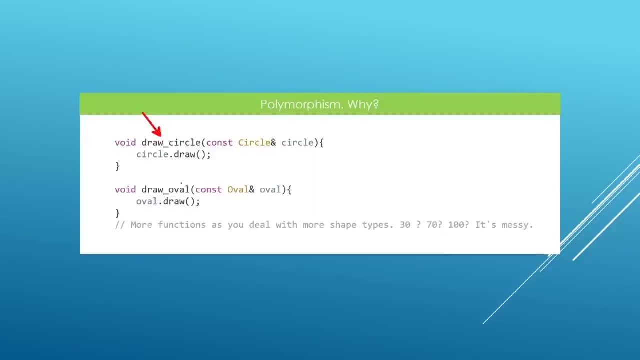 with the current setup we have, we would set up a draw circle method. if we want to draw a novel, we would need to set up a draw over method and this will call our circle draw method and this will call our oval draw method. this is going to do what we want, but try to think about this: if we have 100 shapes in our 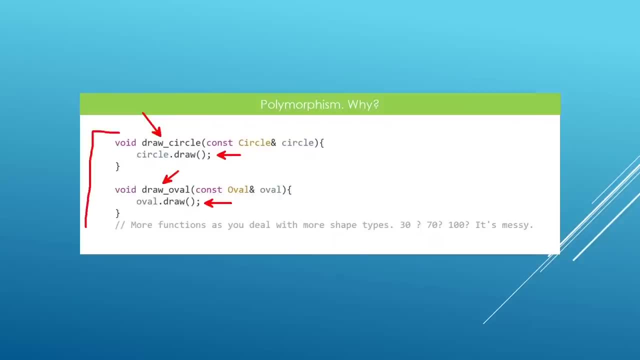 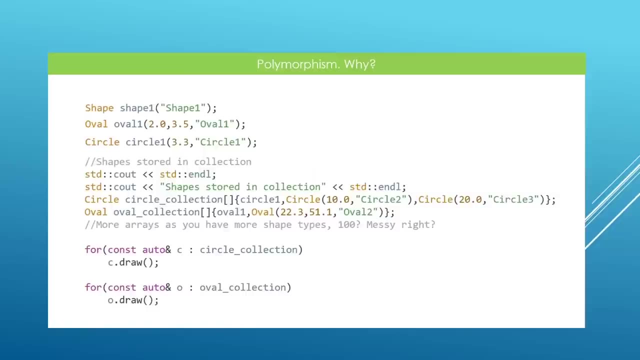 program, we will need to set up 100 such methods, and this is a mess. I don't think you want to do something like this, and we have another simple case that I want you to consider. suppose we want to store all these objects in collections and we're going to use an array to try and drive this point home here. if you, 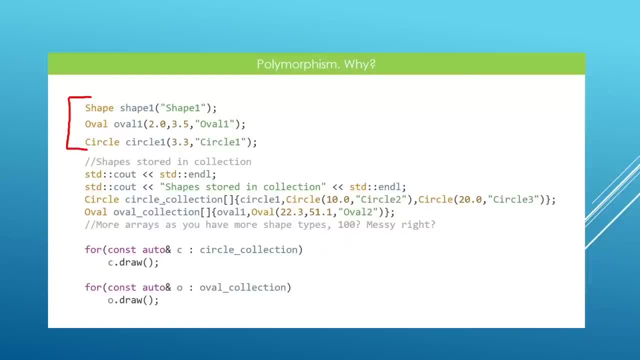 want to store these guys in collections, we will need to set up different collections because, as we have it now, we can't store different types in an array. so what we would need to do now is to set up an array for circles and set up an array for ovals, and do more collections for different kinds of. 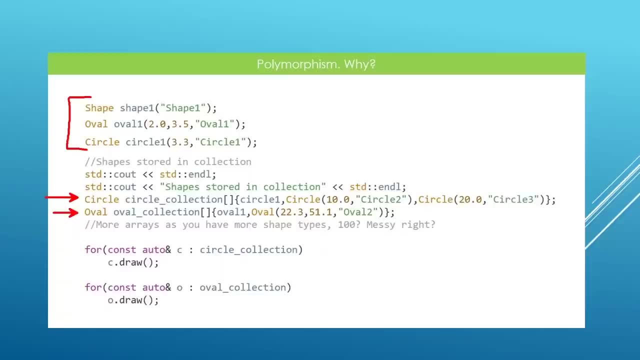 shapes that we support in our program and if we want to draw them, we have no choice but to set up different kinds of loops, and each of these loops is going to be looping on each of these collections here. hopefully, you can see that this is bad design. we don't want to do this. we want to set up something that. 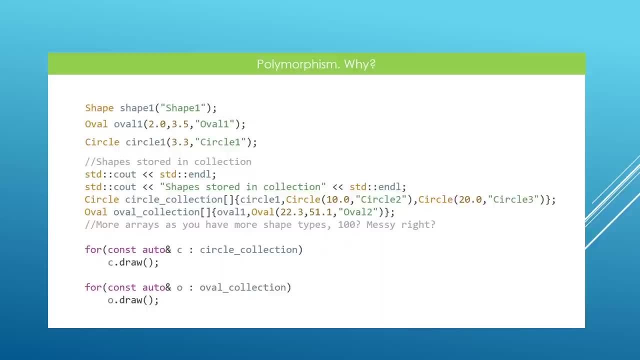 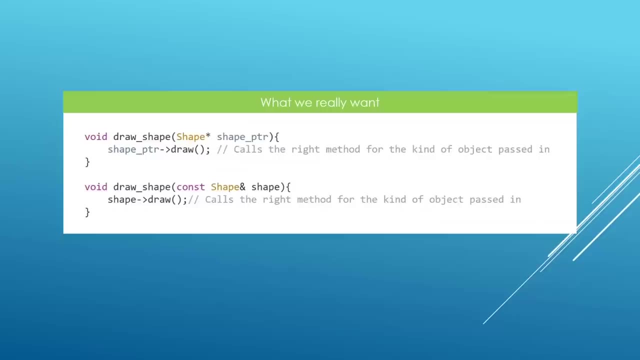 is really easier to manage in our program and polymorphism was- and polymorphism in C++ was designed to be a little bit more complex than what we designed to exactly solve this kind of problem. what we really want in our C++ programs is to set up one Joe method, for example. we can give it a base. 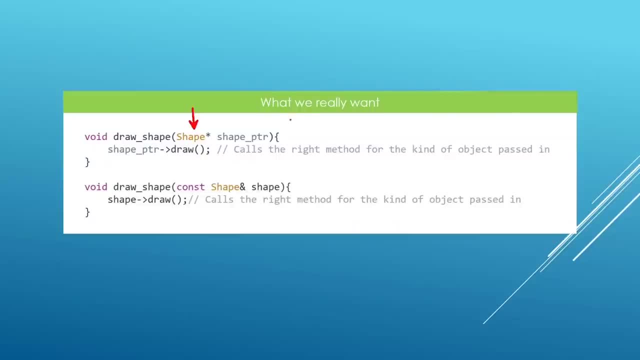 pointer and it doesn't matter which kind of object we pass it when we called us, we will get that method to be called at runtime when we actually need to draw this shape. if we pass in a circle, this is going to draw the draw method on a. 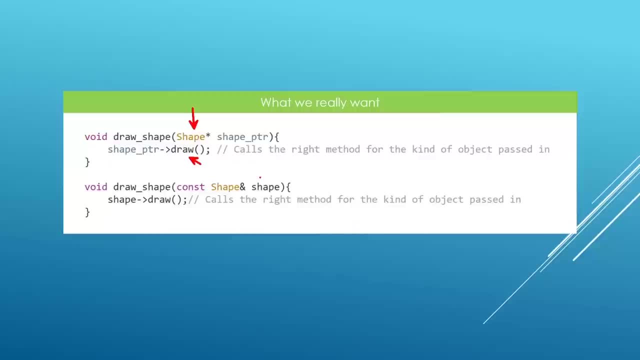 circle. if we pass in a novel, it will call the draw method on our oval object. if we pass in a rectangle, for example, it is going to call the draw method on our rectangle object. this is what we want. we also want the same kind of setup if, for example, our functions are taking: 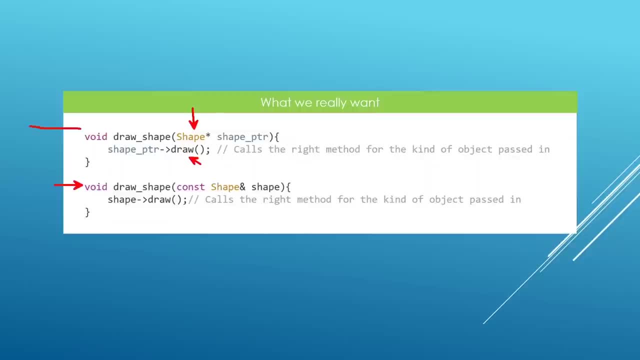 reference, and this is what we're going to get. this is what we want with polymorphism, and this is really going to improve on the design that we had earlier, when we needed to set up a specific method for each shape and we would end up with hundreds of draw methods. 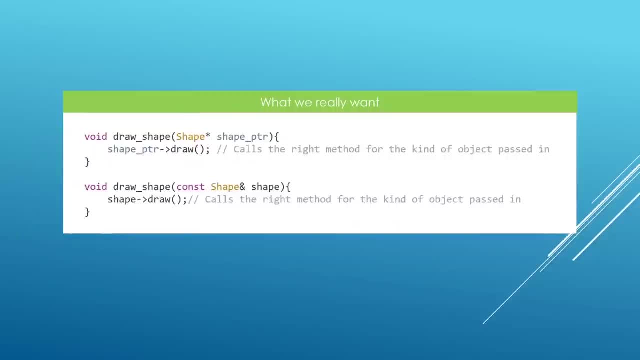 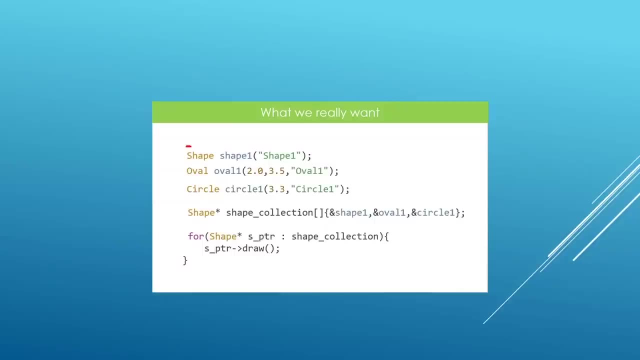 that's really bad. it's not manageable. this is also going to solve our problem with collections. we really need to set up one collection which is going to be taking into account all the shapes that we manage in our inheritance hierarchy. so the setup we do is something like this: we're going to set up an array that 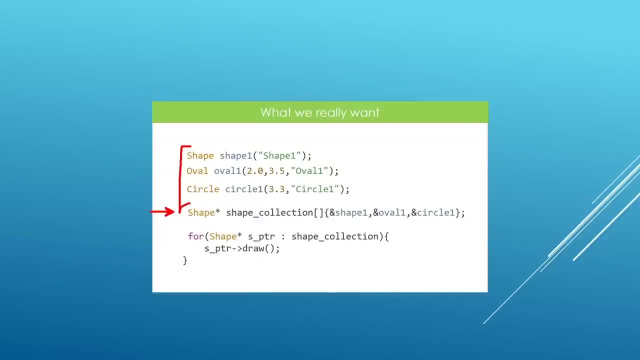 is going to be storing pointers to shape and we can store in the address of a shape, we can store in the address of a novel, we can store in the address of the circle because, if you really think about it, a circle is a shape and always a shape, and the shape is a shape. so this 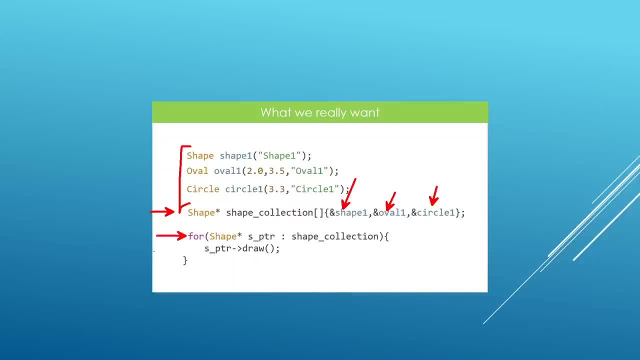 is going to work. and when we get to loop through this collection and call the draw method for the first item, here we will call the draw method on the shape. for the second element, here we will call the draw method on the awful object. and for the third element, here we will call the draw method on our circle object. and 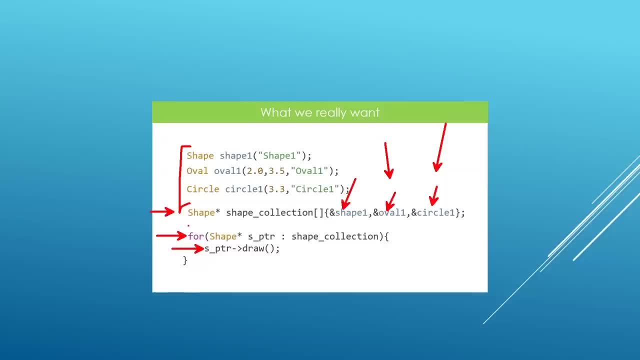 we will draw a shape, a novel and a circle with just one loop, and this is really cool. this is the design we want. now this is not the default behavior we get in our c plus plus classes. if we set up an inheritance hierarchy with our drone methods, what we get by default. 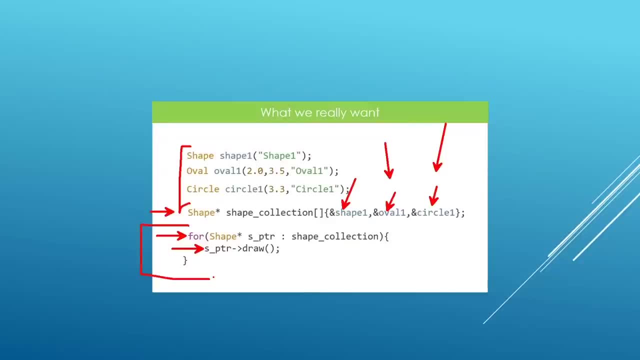 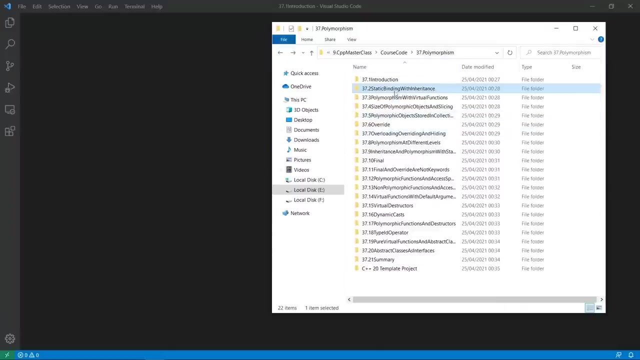 is static binding, but we will see how we can get dynamic binding, all polymorphism- in the next lecture. for this one, we're going to explore static binding and we're going to head over to visual studio code and play with this a little more. here we are in our working folder, the current project. 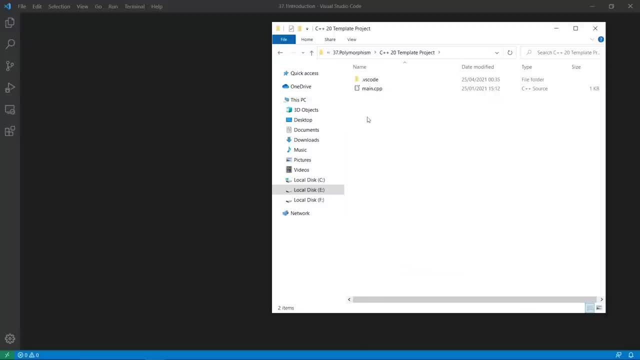 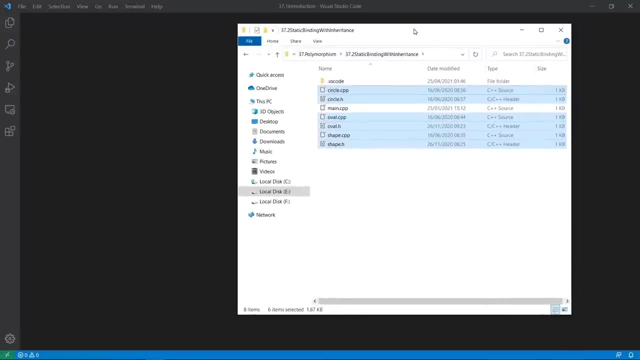 is static, binding with inheritance. we are going to grab our template files. this is going to be our starting point here. we're going to put in these files and i am going to put in our classes to save time. if you want, you can download these classes from the attached resource section on this. 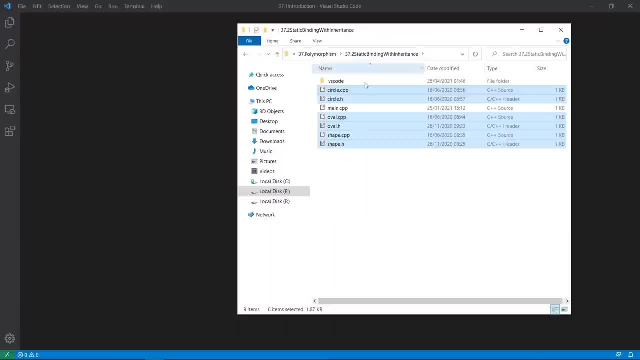 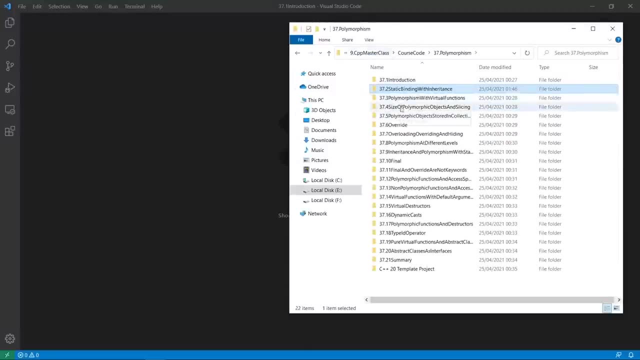 lecture. you're going to find them and you can use them as a starting point. this is going to save us a few seconds, because we don't really want to type these classes. you already know how to create classes if you made it this far in the course, so i am going to drag this and drop here to open in. 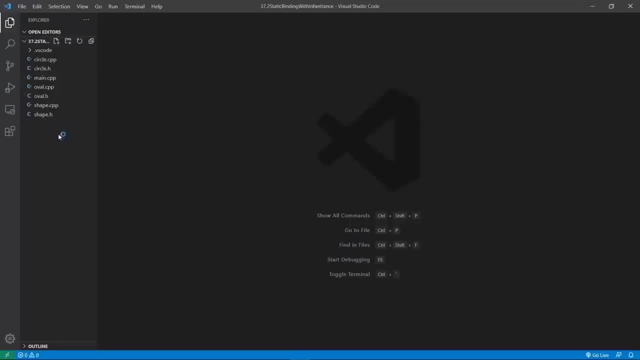 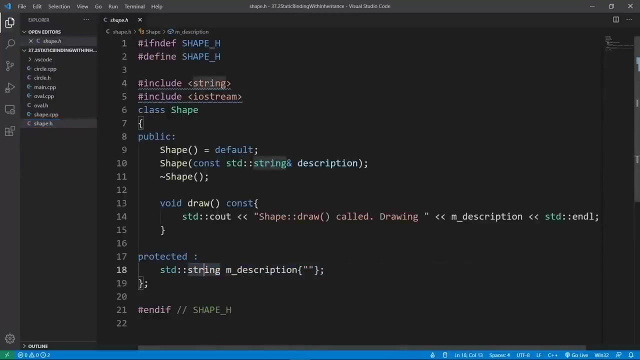 visual studio code, and this is going to give us a good starting point. here we have a base class, which is our shape class. it is going to have a simple member variable, which is going to be the description. one thing i think we need to improve on this is to use a string view to pass our 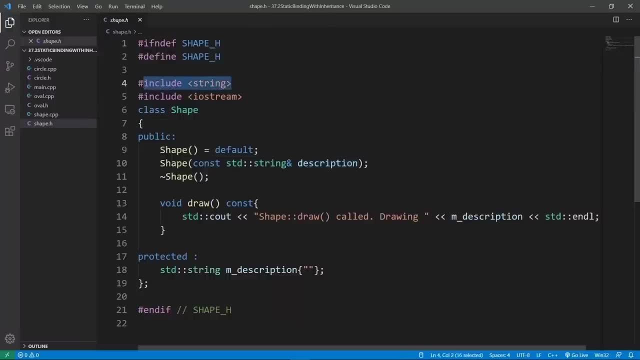 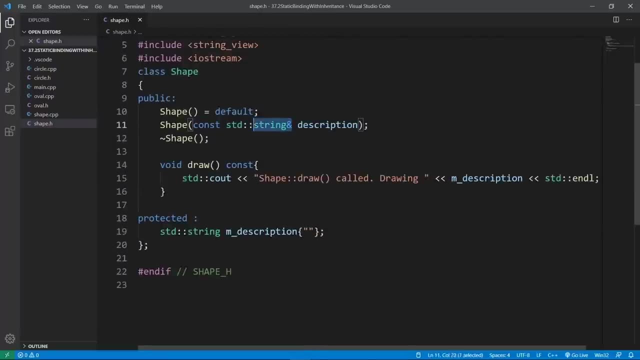 parameter here. so let's include string view. we can include that here. we're going to say include string view, because we are using modern c plus plus and we're going to change this to be an sdd string view by value. you can do this, okay, so we have our class here and we have a draw method. 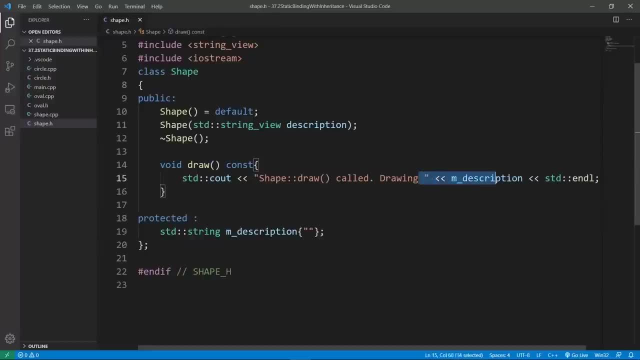 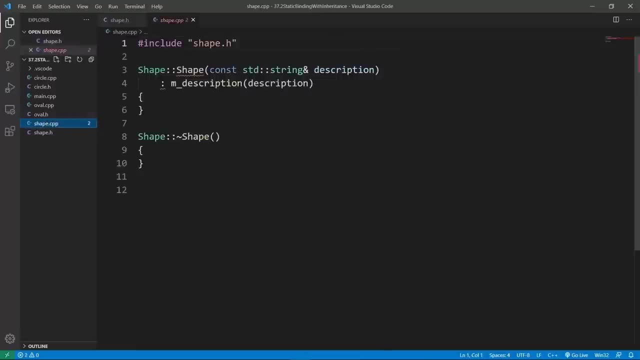 which is really not going to do anything special. it's going to just print the description here and we're going to see it printed out on the output stream. if we look at the cpp file, we just have an implementation of our constructor and you have a destructor. we're going to fix a. 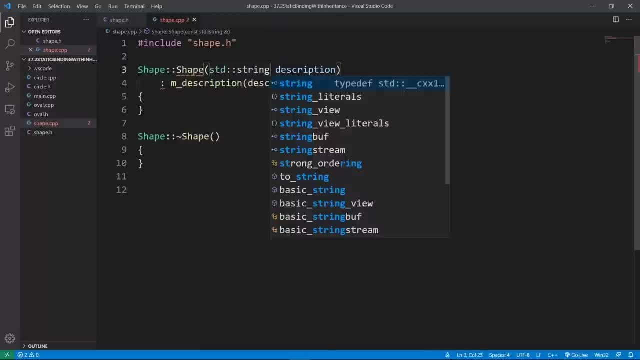 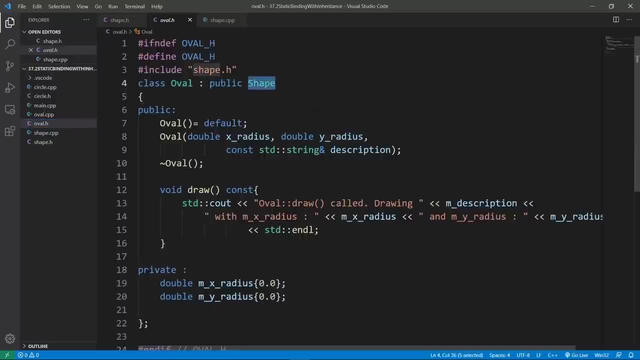 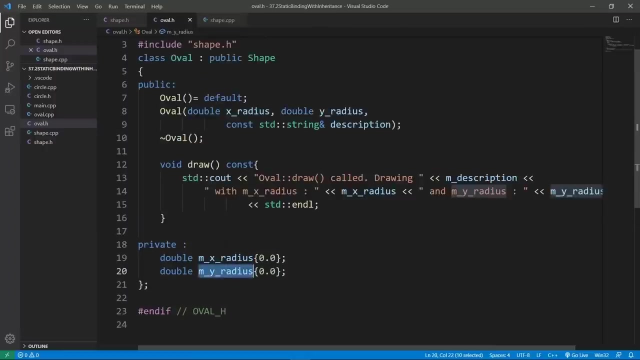 our parameter here to make it an std string view. let's look at our oval class. it is going to be deriving publicly from shape and we have a bunch of member variables here, two to be exact. one is going to be the x radius, the other is going to be our y radius. we have a constructor here which. 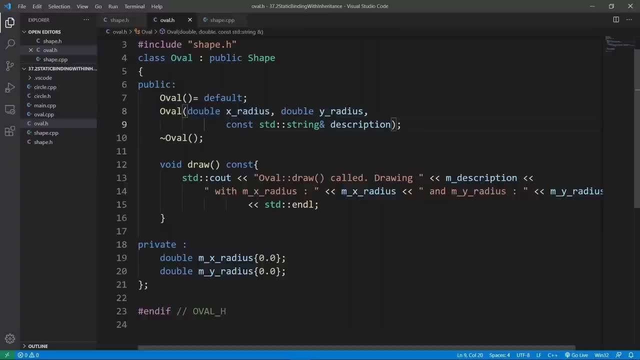 is going to be taking three parameters: two parameters for the data for our radius here, and we have a third parameter which is going to store our description data. we're going to also change this to bstd string view and this is going to do. we have a draw method which is going to 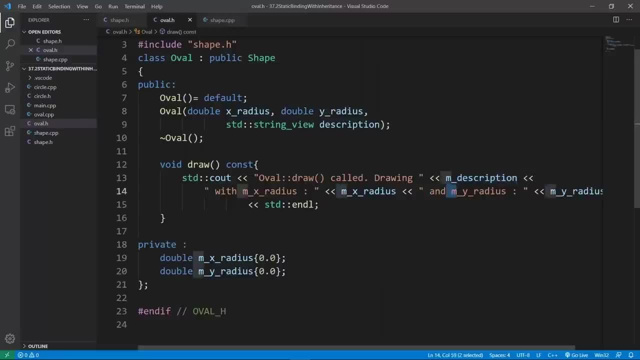 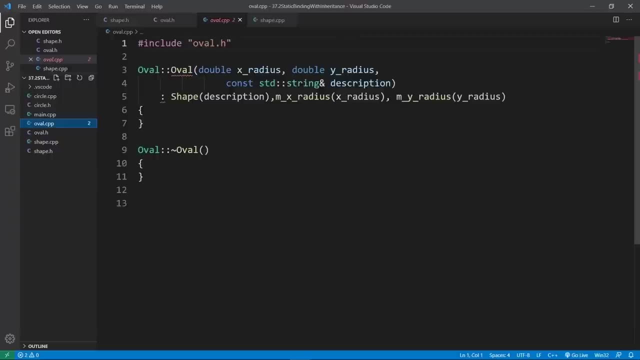 be printing the description and our radius data, and this is really it. we don't need anything fancy here. let's look at our oval cpp file. it is going to have the implementation for our constructor and our destructor here. we just need to change the type for our description here and make this an std string view. 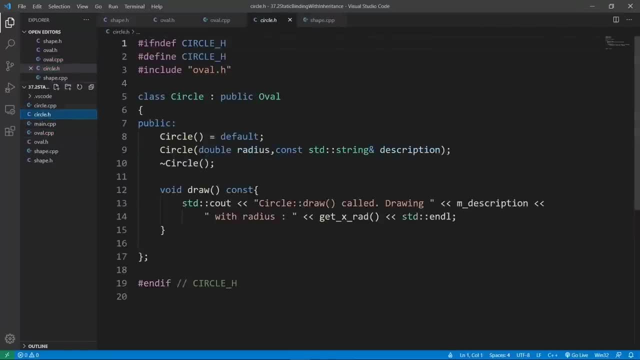 let's do this and we will look at our circle class, which is going to be inheriting from oval publicly. it won't have any member variable because it's just going to forward the data to the oval part of us. it doesn't really need to do any other specialization, but what we need. 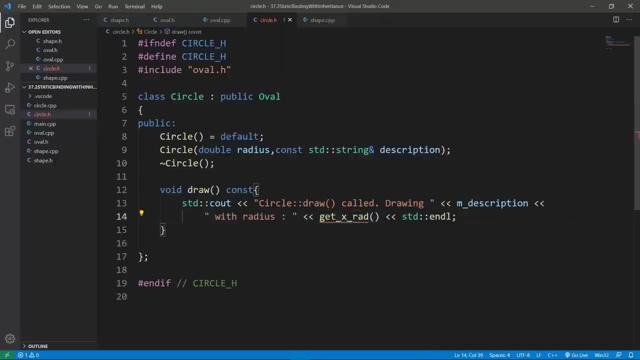 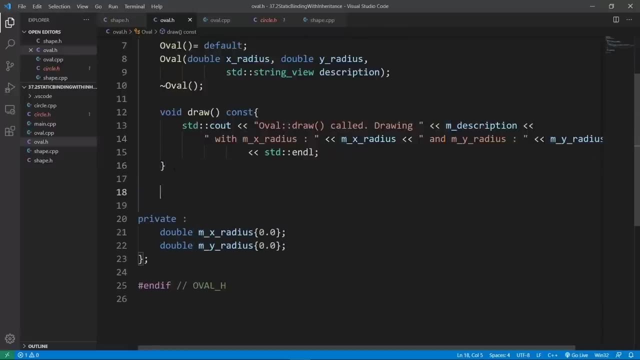 is a method which is going to return the radius, because we want to print that here so we can head over in our oval class and set up a protected section, which is going to give us these methods here, so i am just going to put them in here. 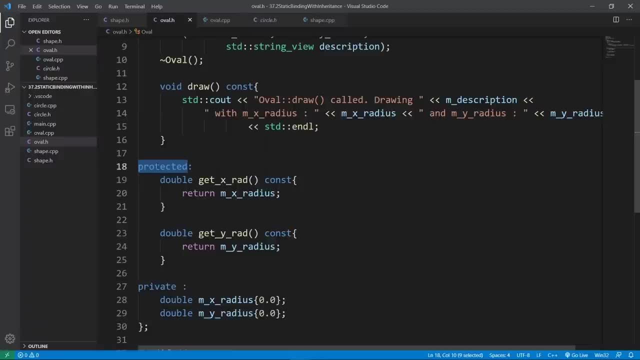 to save on some time. it is protected because we want this to be usable in derived classes, but we don't want this usable from the outside. this is the setup we can achieve by making these guides protected here. get x rad is going to return the x radius. get y rad is going to 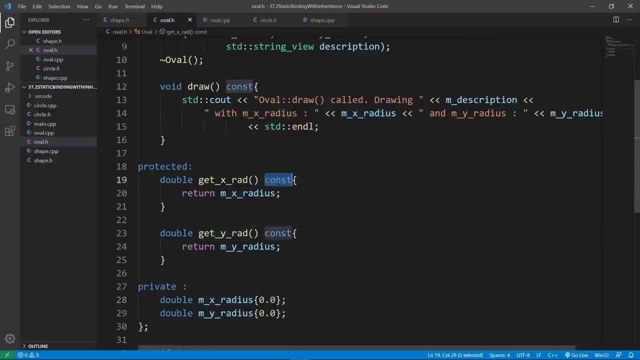 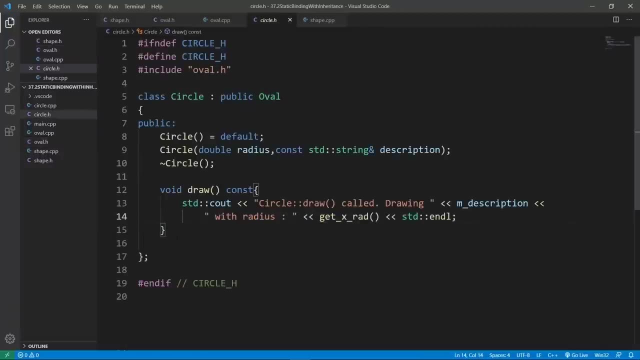 return the y radius. they are cost because we don't intend for this to modify our object and if we go in our circle class, this is going to work. now we will be able to print our information on our circle object and we will see on our output stream. if we look at the implementation, 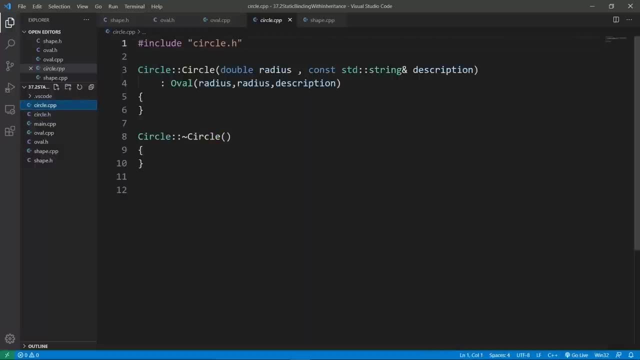 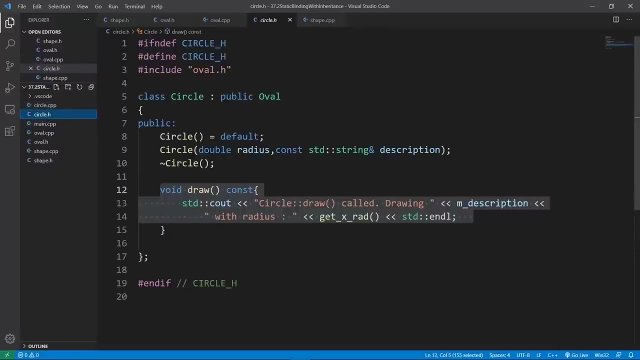 of our circle class. it is nothing complicated. it is just going to take the double radius and it is going to forward the data to the oval part of us. our description here will need to change to take into account that we want to use std string view here, so let's change this to be std string view. we can do that and we are going to head over in. 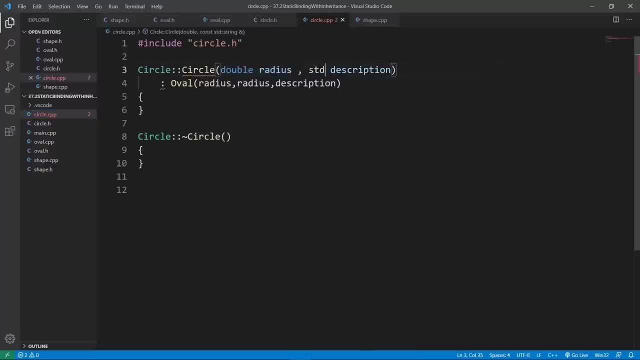 our cpp file and change that as well. std string view. we can do that and now our classes are really complete. we can head over in our main cpp file. we can clean that up a little bit and we're going to see what we need to do here. we are going to include our classes, so we're going to include 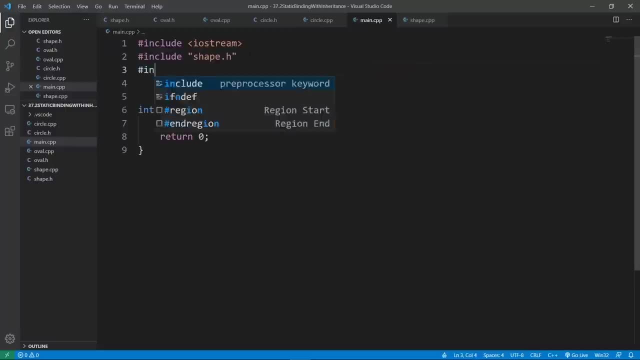 shape. let's do that. we are going to put in oval, let's do that- oval dot h and we are going to put in circle and we are going to create objects of these classes and try to print their information. so we're going to set up a shape called shape one. we're going to set up a novel called oval one. 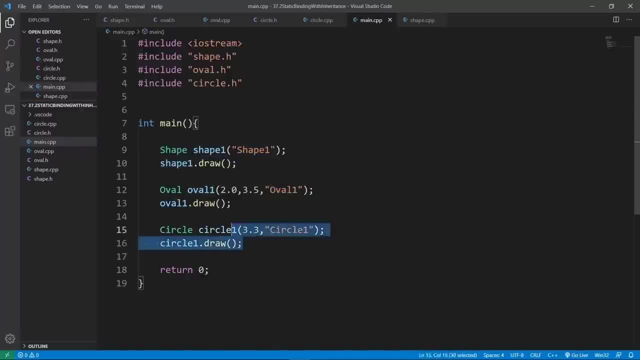 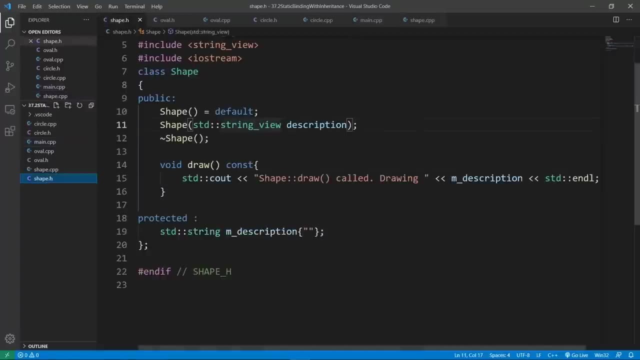 we're going to set up a circle called circle one and we're going to see what kind of information we see. try to call the job method again in shape. the drill method is just going to say that we are calling shape joe in oval. we are going to say that we are drawing an oval and we're going to 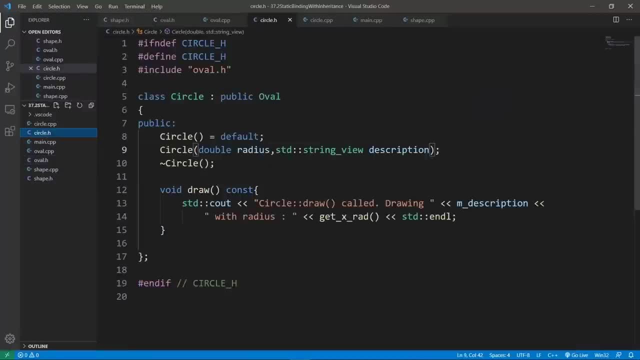 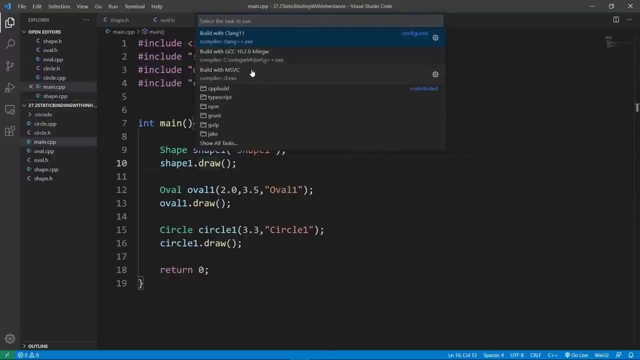 say the description and the radius in circle. we're going to say that we are calling the drill method on a circle object and say the description and the radius here. this is the information we want. so we are going to try and build this program using gcc, our favorite compiler. you can really 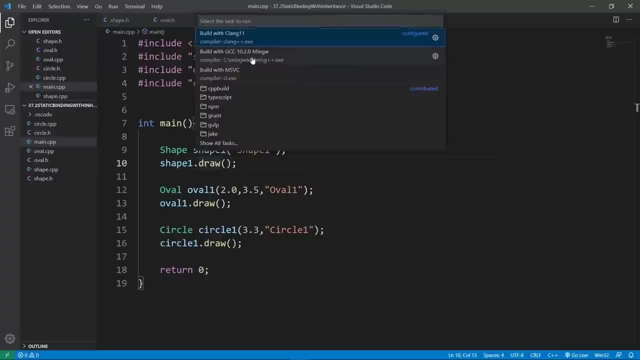 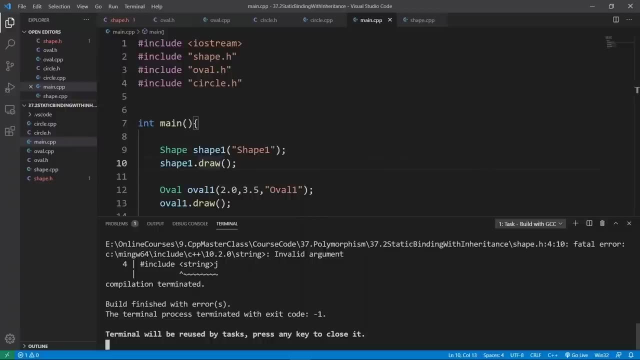 use any compiler you have your hands on, but we are going to use gcc here because it is our favorite and we're going to have a bunch of errors. what it is that we have here. what is it that we have here? let's go in shape header at line 4 and see what we have, and we have a j here that we don't want. 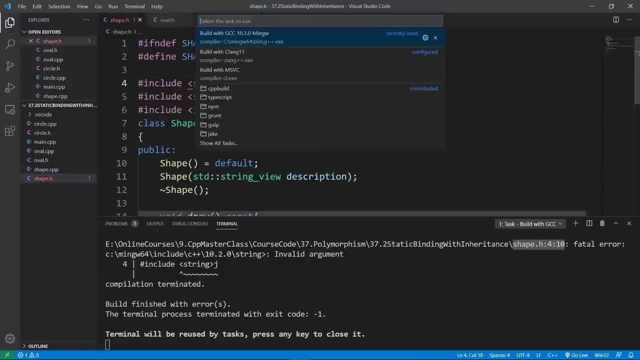 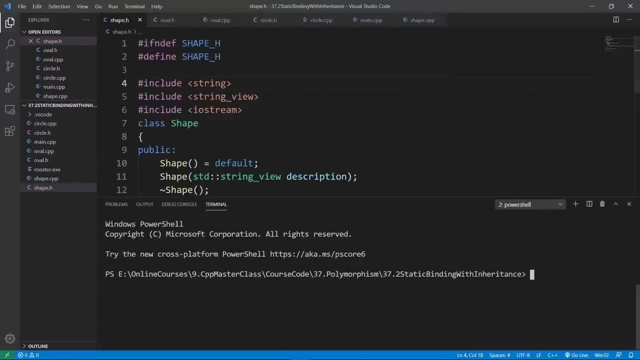 let's take this out and we're going to build it and we're going to pass this through gcc and the build is going to be good. we can bring up a powershell window to write our program. let's run rooster and we're going to see that shape joe was called drawing shape one. 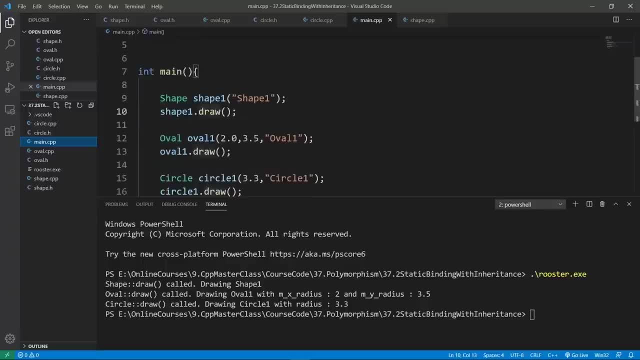 you see, we have just created shape one here and we are printing its information. we are going to call the oval draw method and we're going to print the information on that. you see that it is all for one here and we're going to put out our radius data. x radius is going to be 2, as we specified. 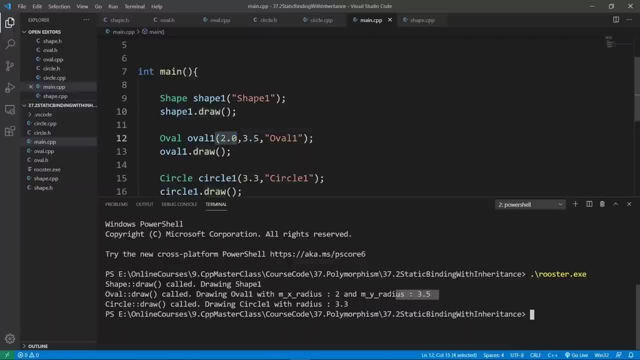 here, y radius is going to be 3.5, and this is going to be 3.5, and this is going to be 3.5, and this is our information. we are also going to call the draw method on our circle object. this is what we get. 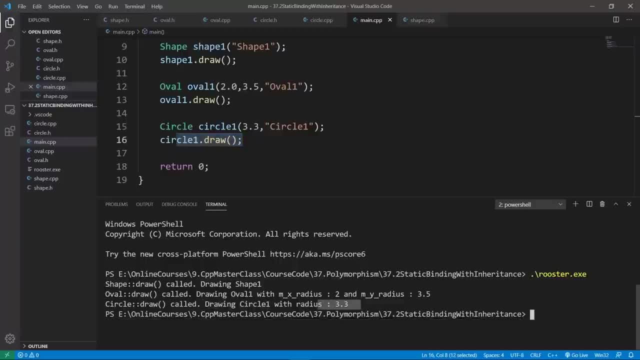 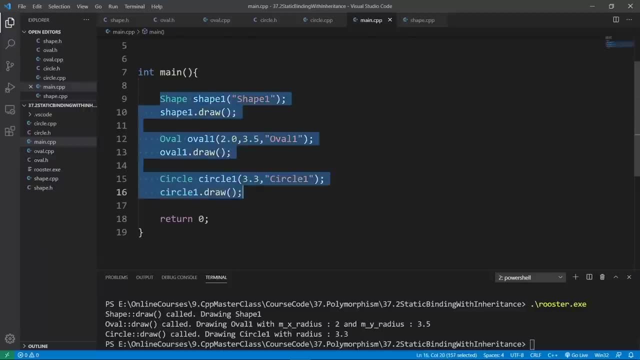 and we're going to say we are drawing circle one and the radius is going to be 3- 3. this is our information here. but we don't want to go through direct objects to manage our data here. what we want is to either go through base pointers or base references. so we are going to set up 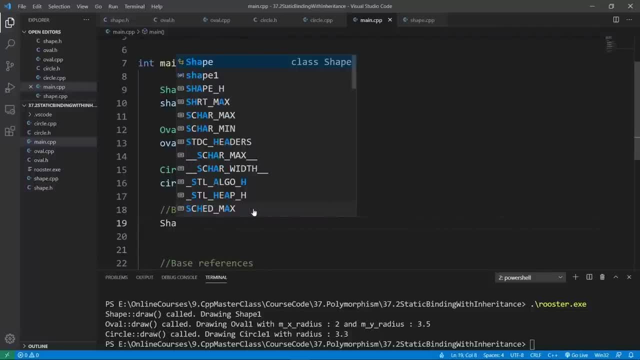 a shape pointer. let's do that. we're going to say shape because that's our base class, and we're going to say shape ptr to represent our pointer and we're going to store in the address of shape one. you can do something like this and to really see what is happening, we're 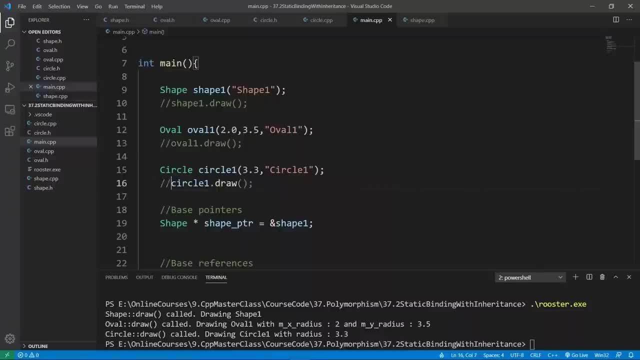 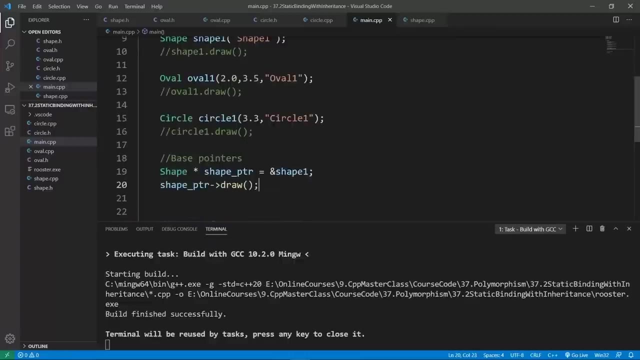 going to comment out our calls to draw methods here and we're going to see what happens. so if we say shape ptr and call the draw method, we can do that. let's try and build our program. we're going to pass this through gcc. you're going to see that it is going to work and it is going to do what. 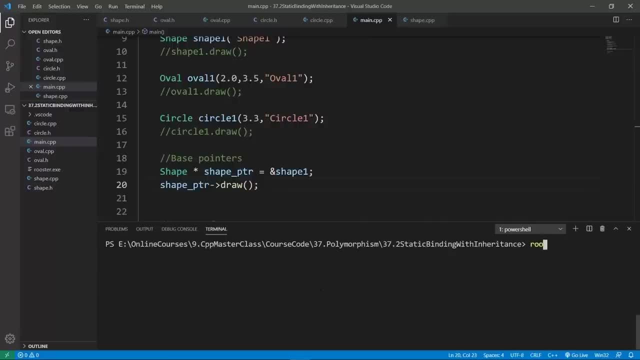 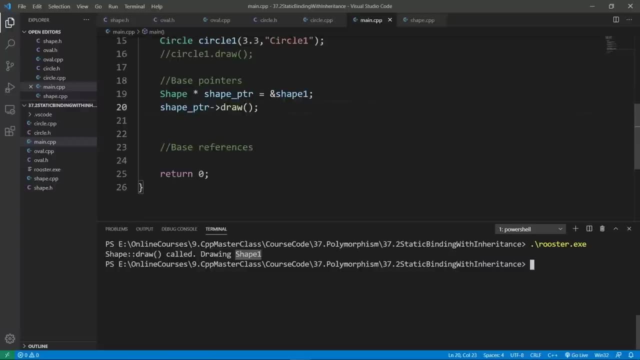 we expect. if we run this program- here you can clear and run roaster- we're going to see that shape draw was called and we are going to be drawing shape one here. this is what we expect. but if we go down and say we don't want to call the draw method here, we are going to store in. 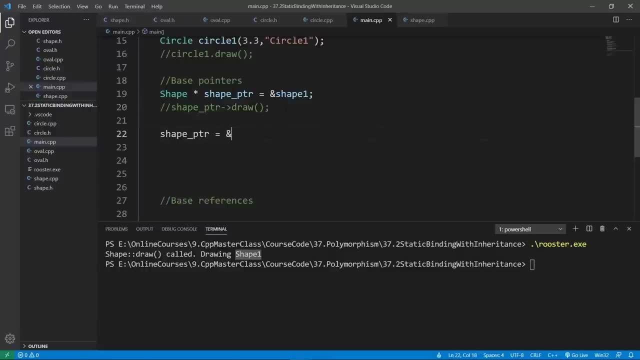 let's say shape ptr and we're going to store in the address of our over one object and we want to call the draw method here. now, if you do this, as we saw in the slides, what we really want is to get the draw method on our actual oval object called and if we will, for example drawing, 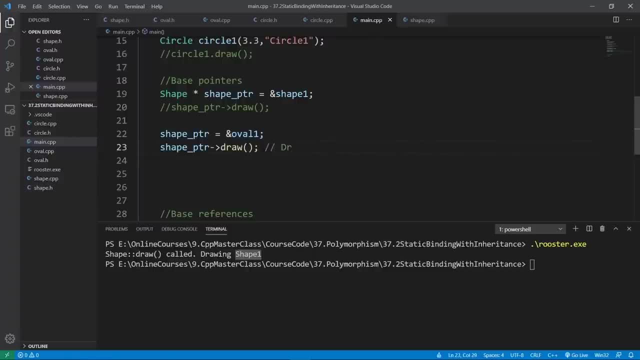 things on the screen, we would draw a novel. this is what we want here, but this is not what we're going to get. you're going to see that we still get the job method from the shape class called, and it is going to and it is going to say: drawing over one, let's try. 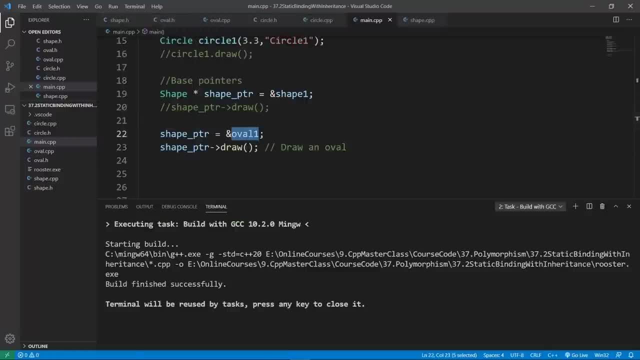 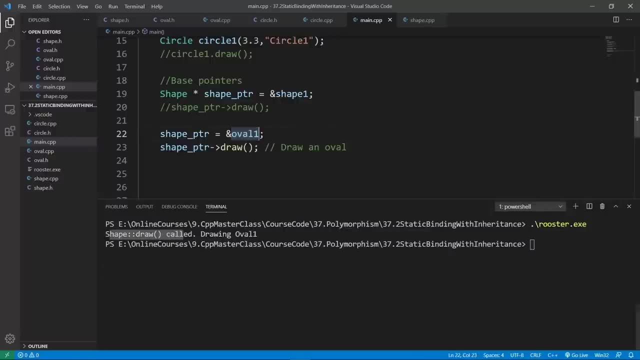 and see if we can get the draw method on our actual oval object called and if we will, for example, draw- and I really want you to see this- so the world is good, we can clear and run roaster. you're going to see shape draw even if we are storing again a novel object. so this is the 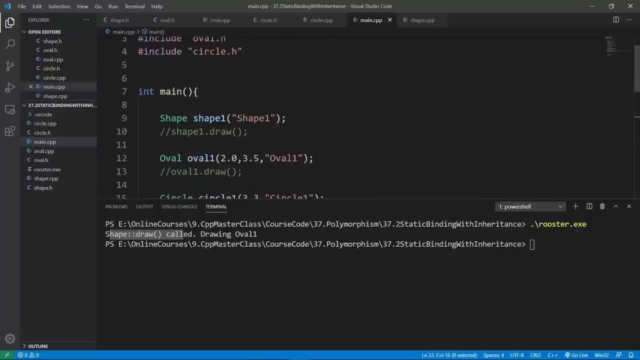 default behavior we get, and this is static binding that we get by default in our inheritance hierarchies. so what the compiler is really going to do here, it's going to look at the type of the pointer that we have here. it is going to say: I have a pointer that we have here and it is going: 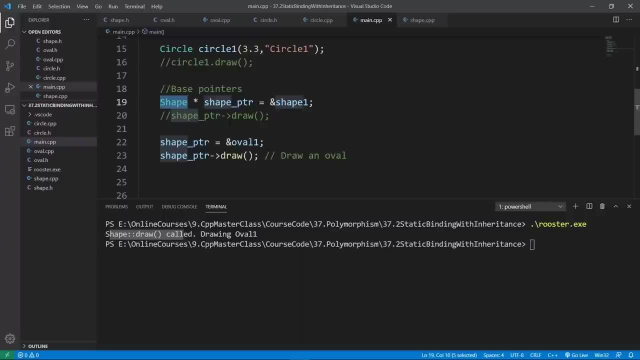 a shape pointer. so i am going to call the draw method on the shape type that i have in my pointer here and we are going to see that this is calling the draw method on our shape and this is not what we want in most cases. we are going to see that we get the same behavior if we store in a circle. 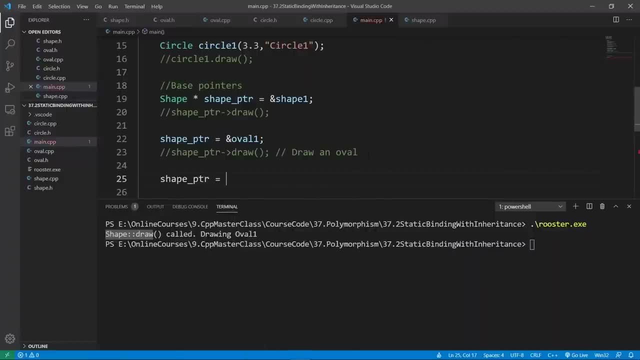 object. let's do that. we're going to say shape pointer and we're going to store in the address of our circle one and then we're going to call our draw method on our shape pointer again, this is going to draw a shape, it's not going to draw a circle. that we really are managing with our base. 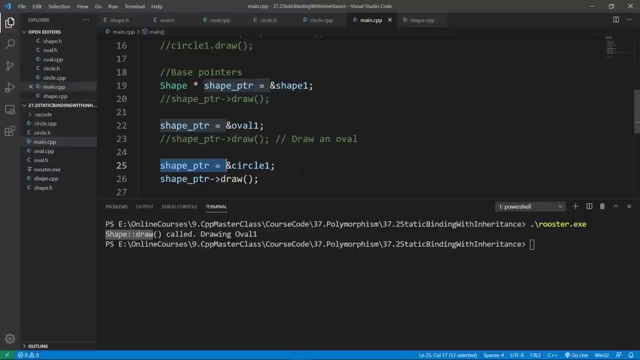 pointer here, and some of you must be thinking: why are we able to store circle pointers, for example, in a shape? well, a circle is a shape according to our inheritance hierarchy. if we take a closer look again here, you can see that we have the same structure we add inside our inheritance hierarchy. 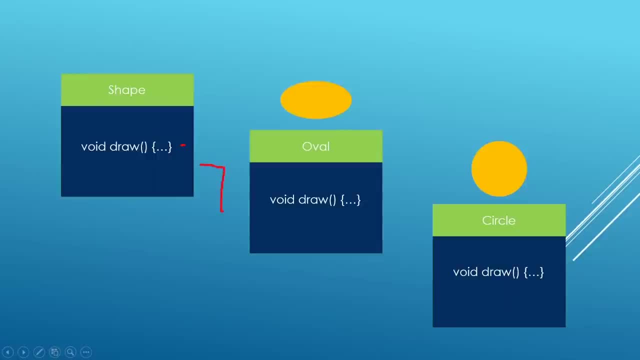 and some of you must be thinking: why are we able to store circle pointers, for example, in a shape? going to see that oval is going to be inheriting from shape and circle is going to be inheriting from oval. so, from what we learned in the last chapter, oval has a shape, coordinate and circle. 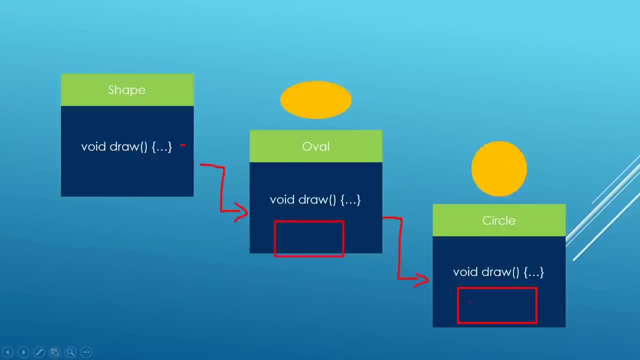 has a novel coordinate which in turn, is going to have a shape coordinate. so from this understanding, it shouldn't really be surprising that we are able to manage a novel object with a shape pointer, or the fact that we are able to manage a circle object using a shape pointer. this is why we are 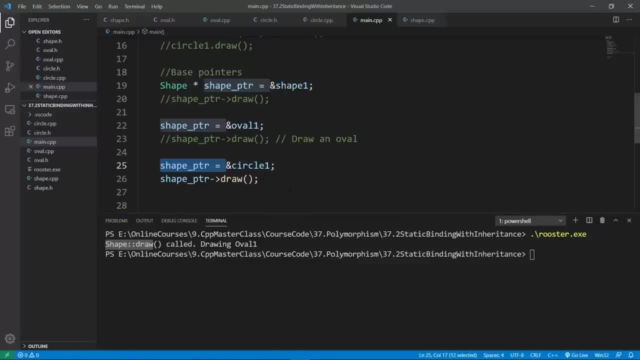 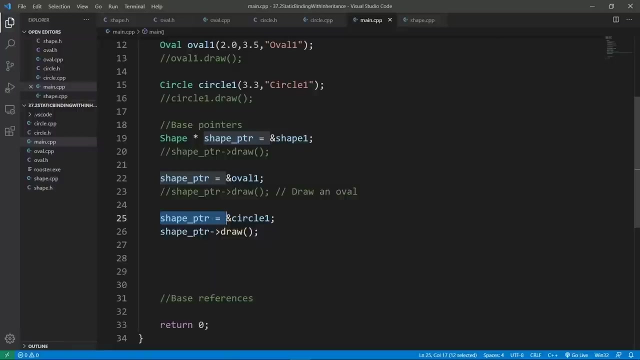 able to do something like this, okay, so i hope this is super clear. but again, we are not getting the default behavior that we want, but we will see how we can achieve that in the next lecture. for now, i really want you to understand you what static binding is all about. and it is the fact that the compiler is going to look at the 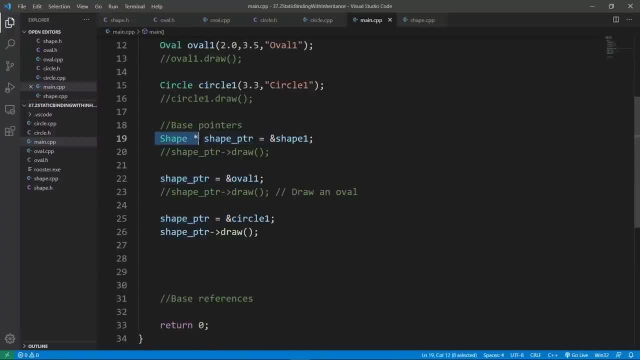 type of the pointer here and use that to decide which method it is going to be calling. in our inheritance hierarchy the compiler, for example, is going to see that we have a circle object stored n at line 25 here, but when it wants to decide which joe version to call it is going to, 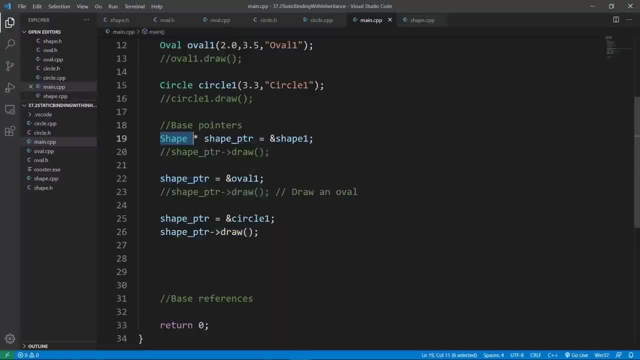 look at the type of this pointer here and it is going to use that to decide which joe method to call, and in this case it is going to call the shape version, because the type of this pointer is shape okay. so i really hope this is super clear here. we are going to get the same behavior if we 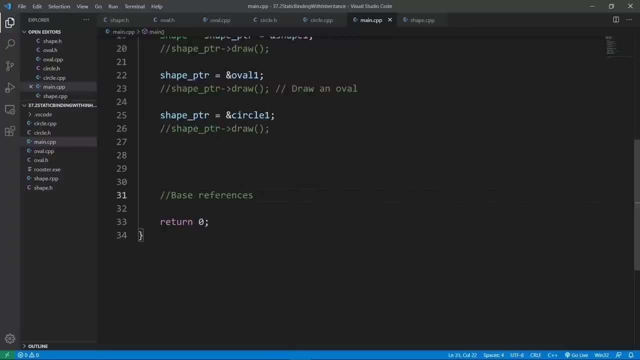 try to manage our objects using references. for example, if we go through a shape reference, let's do that- we're going to say shape reference and say shape ref and we are going to store in shape one, for example, let's do that and we want to call the draw method on. 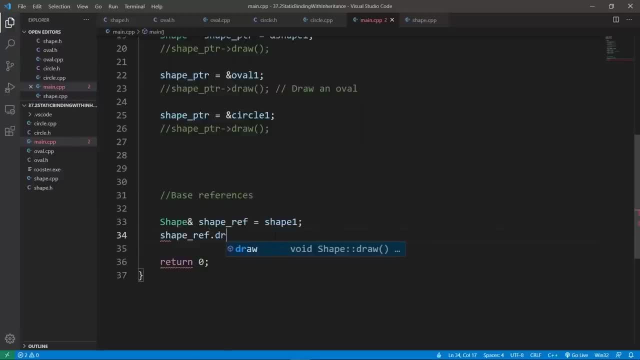 shape reference. let's do that. so let's call the joe method and you're going to see that we will get the shape method called. and this is really making sense because we have a shape object managed by this reference here. so if we build our program, let's do that. we're going to pass this. 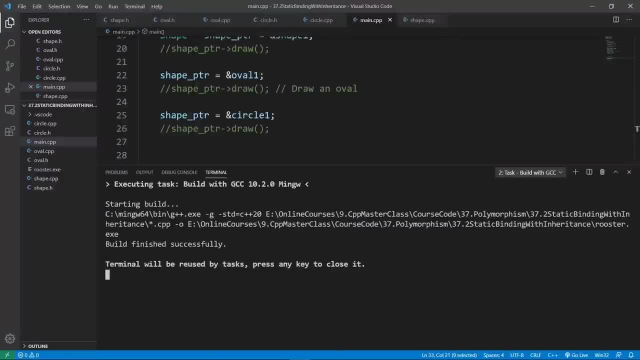 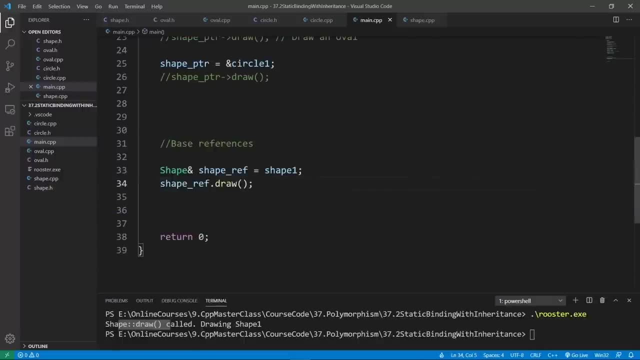 through gcc. you're going to see that we get what we expect. the build is going to be good. we're going to clear and run rooster and we see shape draw called. this is what we want. but if we use this reference to manage a derived object, for example, let's put in oval one- we can do that. 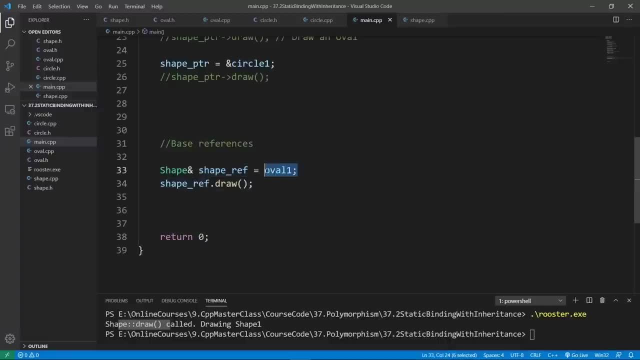 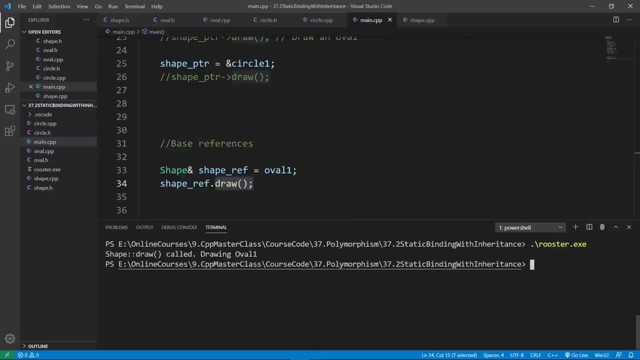 we're going to see that we don't get the most specific draw method for oval here called. we will still get the method for a shape called. let's build and show you this. this is static binding again. okay, the build is good, we can clear and run rooster. we're going to see that shape. 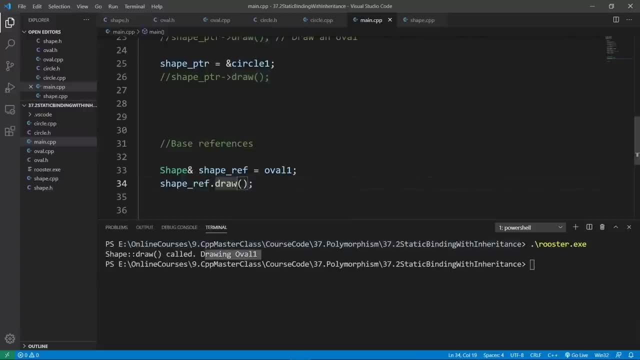 draw. it is joe and we don't get the oval draw method called, we get shape draw method. again, the compiler is going to look at the type of this reference by default and it is going to use that to decide which draw method to call. if we even put in a circle, we are going to get the same. 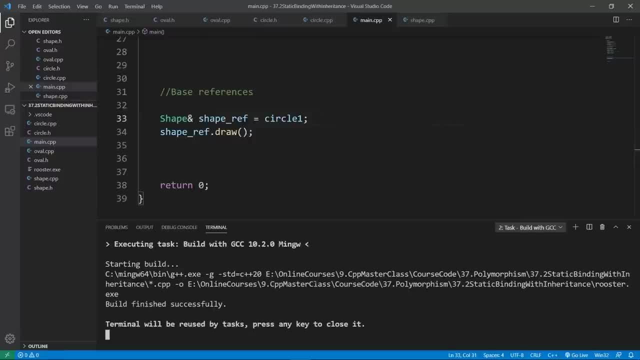 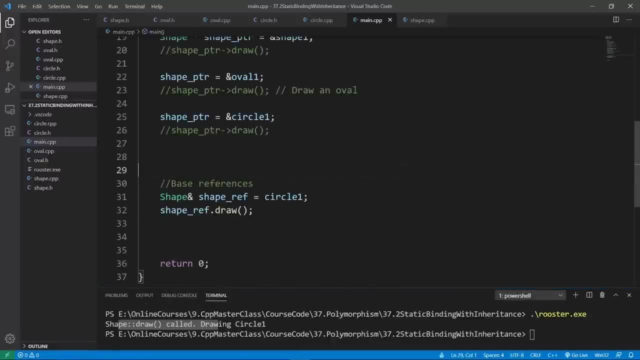 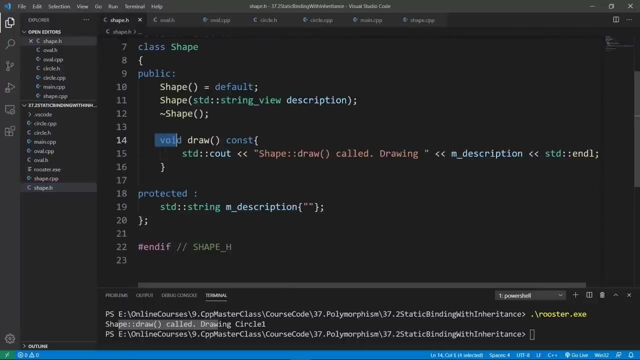 behavior. let's build with gcc. the build is good, we can clear and run rooster. we see that shape draw is called, and this is really not what we want. okay, so this is static binding and it is the default behavior we get if we have an inheritance hierarchy with the same method. 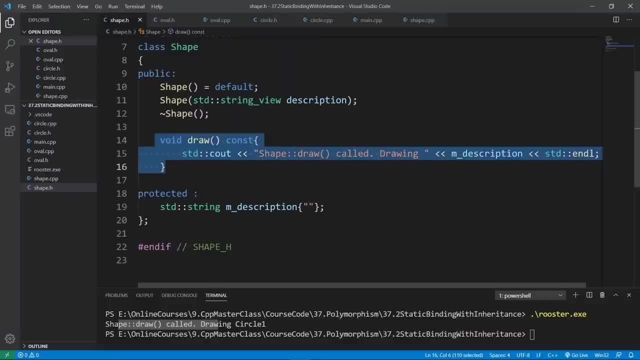 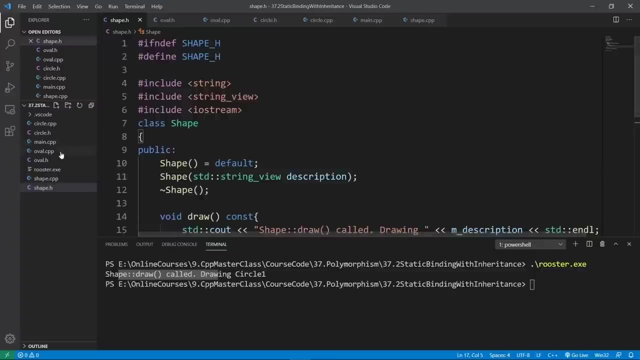 spread across each derived class. we're going to get the shape version called, even if what we are really managing with a shape pointer or a shape reference is a derived object. i really want you to understand this. now let's see why this is really bad design by default in c++, if you happen. 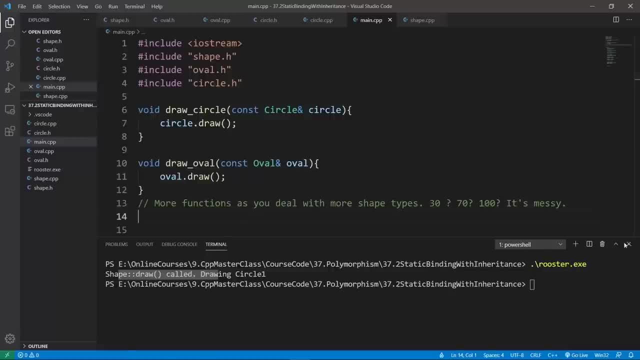 to need to pass shape parameters to functions. for example, we might do something like this: we might need a function to draw a circle, we might need a function to draw a novel and if you happen to have 100 objects you can draw in your program. you have. 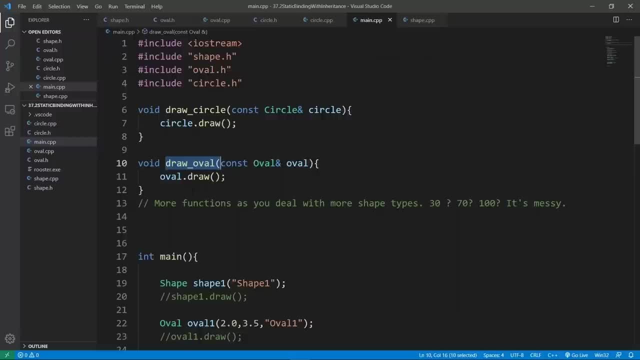 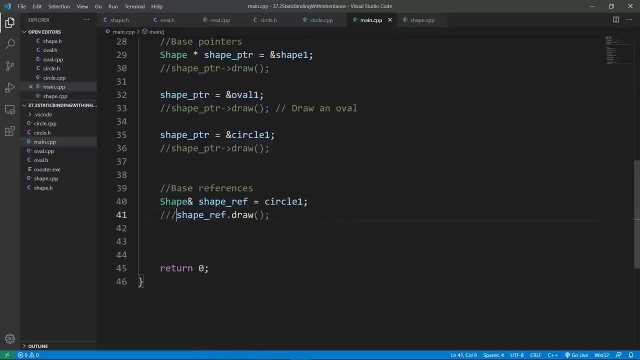 no choice but to set up 100 drawing methods or functions. this is really bad design. you don't want to do something like this. so what you would do in your program, for example, is go down and say drawing. and you would say, for example, draw a circle and pass in a circle and say draw. 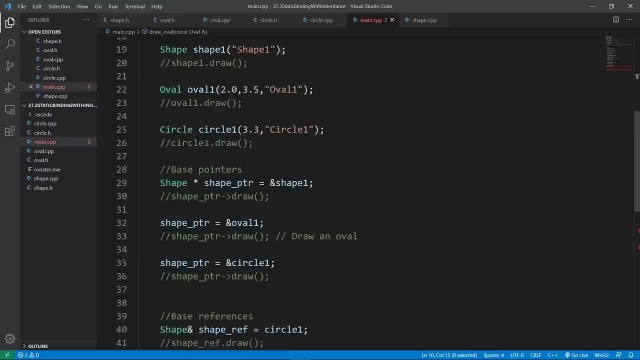 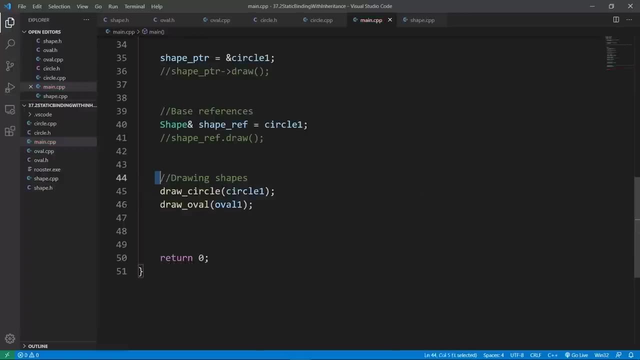 oval. do we have a draw of full function? let's see, yes, we have that. we can go down and say draw oval and pass in our oval one. this is going to work just fine. but hopefully you can see that this is bad design. if you have a lot of shapes in your program, this is going to quickly become. 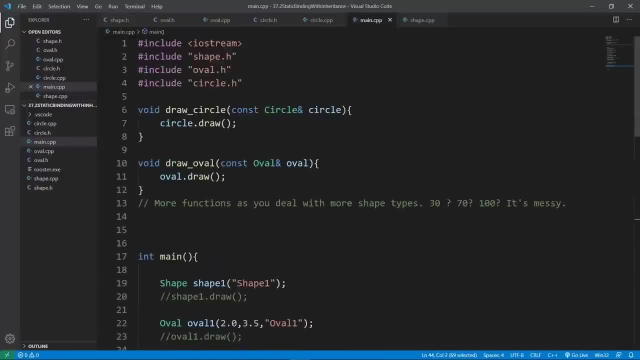 and manageable and you don't want to do something like this. what we want is to be able to only have one method and get to the c plus plus runtime to resolve which one is called that runtime when we get to pass our actual objects, and we will only have one function which is going to 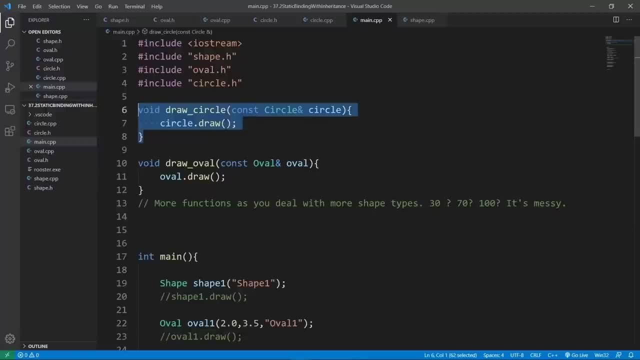 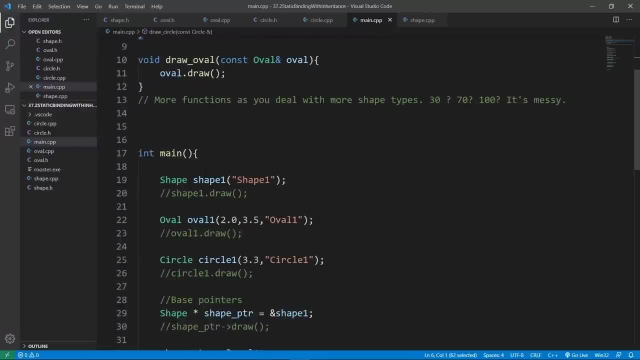 take into account hundreds of shapes that we might potentially have in our c plus plus program. this is going to be much easier to manage and we will actually be able to achieve this in the next lecture, so stay tuned for that. another problem with us is if you happen to need to store these. 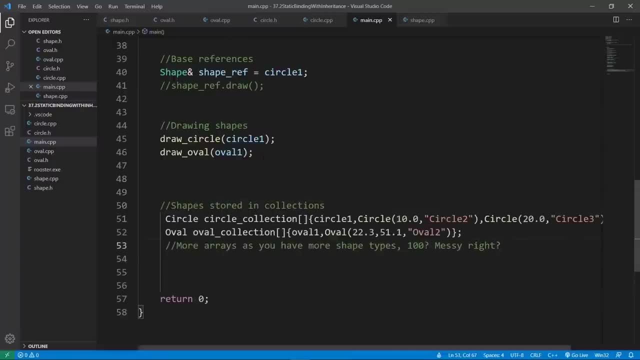 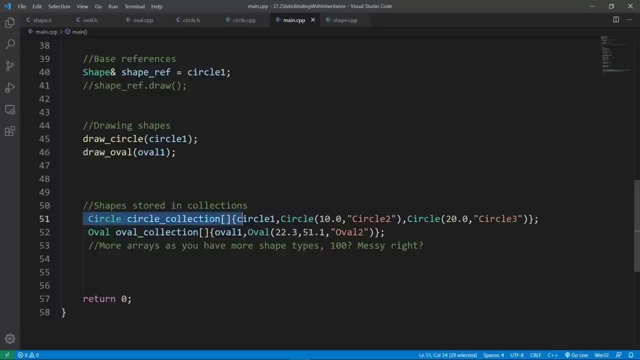 shapes in collections. if you need to set up something like this, you will have no choice but to set up different collections for each type. for example, we might set up a collection for a circle, a collection for oval, and here we are just using arrays to model our collections, and this is really 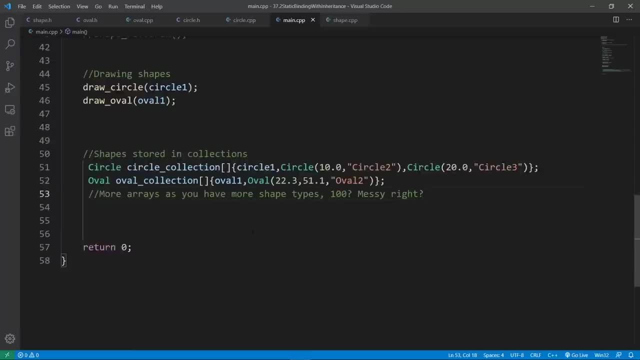 bad design. if you happen to have 100 shapes in your program, you will set up 100 such collections and the only difference is that they are just different types. and this is really bad design because even if they are different types, they are related and they are all shapes in our c plus plus. 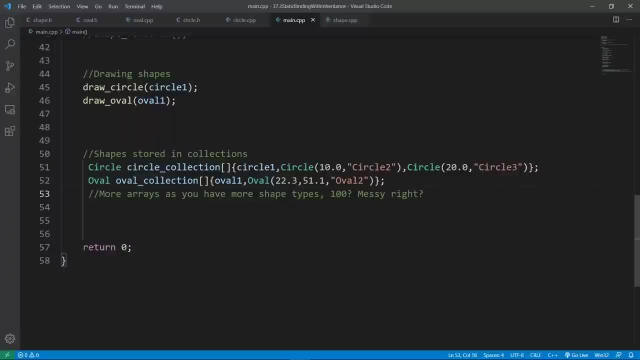 program and what we really want is to set up one collection which is going to take into account all these kinds of shapes that we might have in our c plus plus program, and we will be able to achieve this again in the next lecture, but the whole point of this lecture was to show you static, binding. 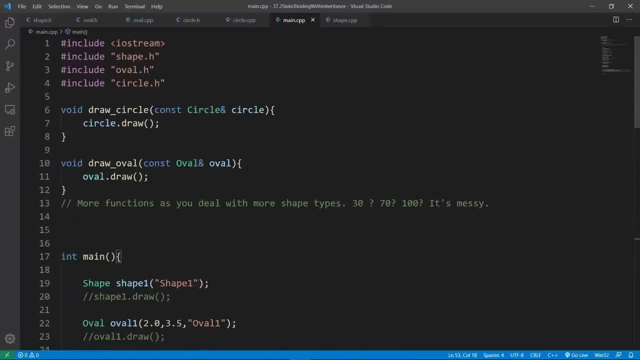 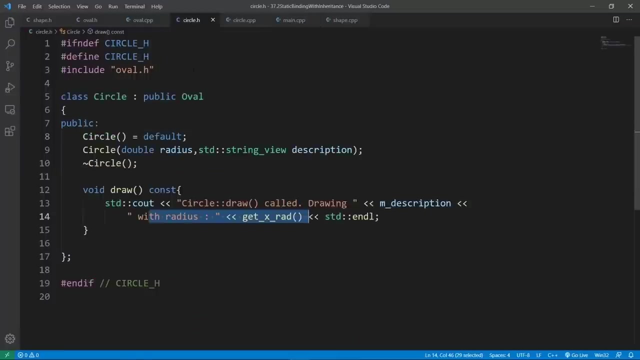 that we get by default with our inheritance hierarchies. static binding may be bad if you really are managing a lot of related objects in your c plus plus program and all of these have the same method that each derived class is specializing, but you want the most specialized. 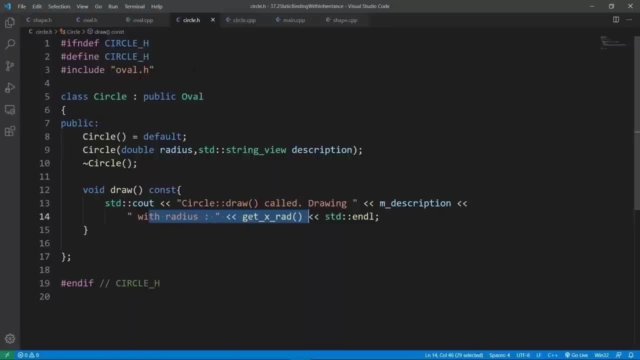 method to be called on, the actual object that you are managing with a base pointer or a base reference. hopefully this is super clear. i apologize, this lecture turned out to be really long, but i wanted you to make this super clear. and everything else we do in the reminder of this chapter is: 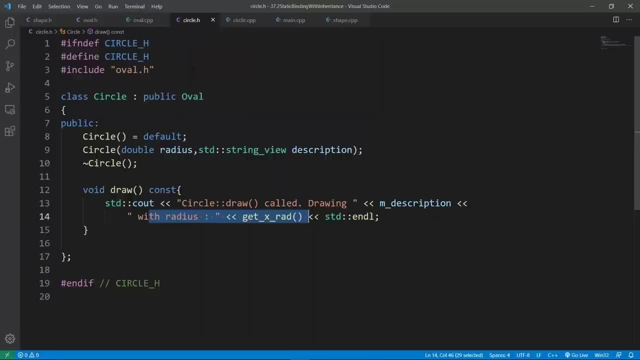 really going to fall in place. so make sure you understand this and if you have a problem, do you ask me. i will do the best i can to help you out. this is really all i had to share in this lecture. i hope you found it interesting. we are going to stop here in this lecture. in the next one we're 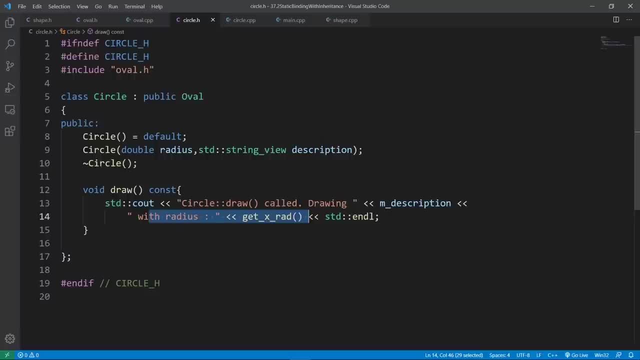 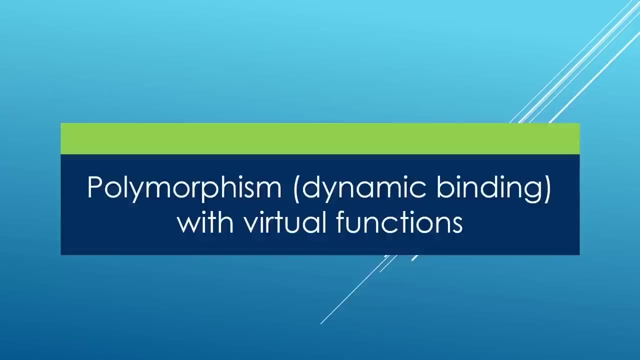 going to show you how you can achieve dynamic binding using virtual functions in c++. go ahead and finish up here and meet me there. in this lecture, we're going to see how we can achieve dynamic binding or polygons morphism, using virtual functions in our inheritance hierarchies. in the last lecture we had a hierarchy. 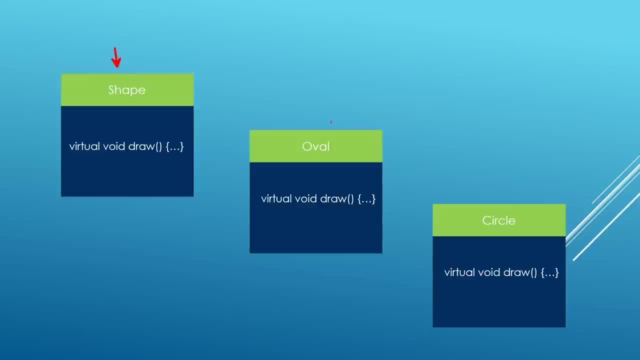 like this, where the base class was shape, we had an oval class which was publicly deriving or inheriting from shape and we had a circle class which was publicly inheriting from oval. and the problem we had was that, if we happen to be managing oval or circle objects using shape pointers or 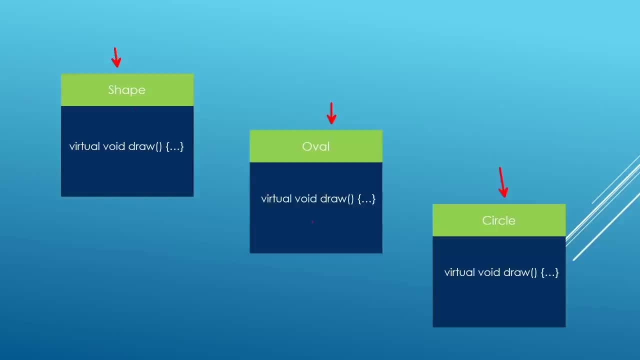 shape references. we don't get the correct methods called if we call the draw method on our base pointer or base reference, and this was really bad and this is something we want in practical c++ programs. i am here to tell you in this lecture that you can just achieve that by doing a tiny modification. 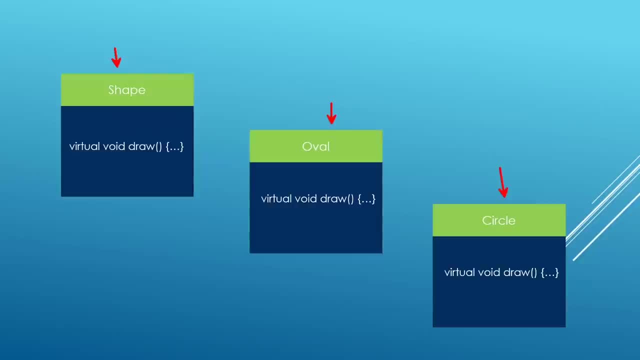 on your inheritance hierarchy. all you need to do is to mark the methods you need to be dynamically resolved virtual, and we do that in the next lecture, and i will see you in the next lecture by inserting this virtual keyword in front of our function. so we're going to do that on our 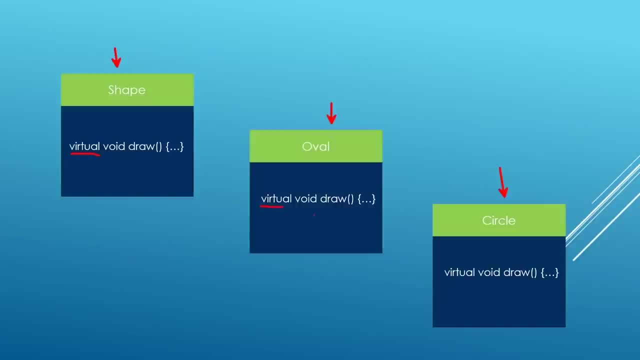 shape class. we're going to do that on our overclass and we're going to do that on our circle class. once we do this, the c++ compiler is going to know i want to be looking at the type of the pointer or reference to know which kind of method to call in my inheritance hierarchy if i happen to be using. 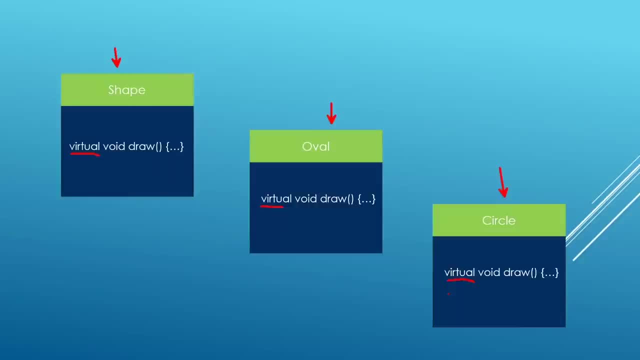 a base pointer or a base reference to manage a derived object and we're going to see that by inserting this virtual keyword in front of our function. we're going to do that on our shape class and we're going to be making this super clear in a minute and if you are lost, please bear with me. 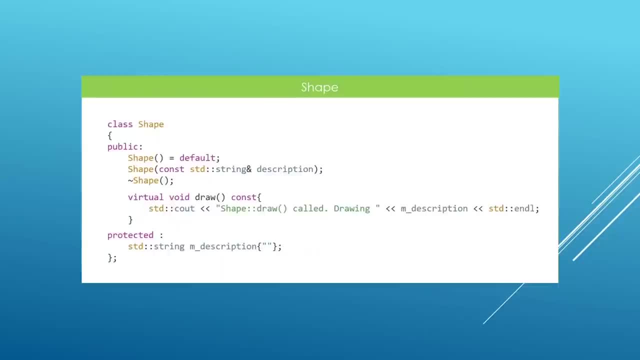 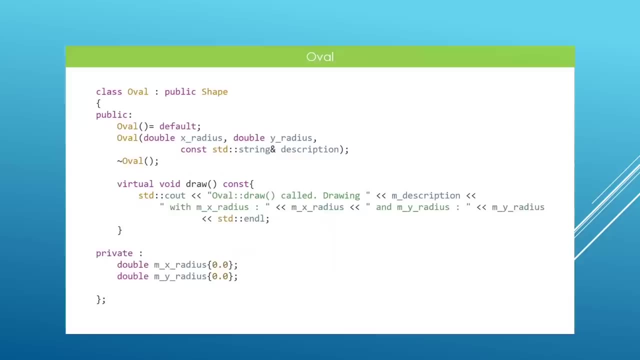 you're going to understand. so let's do this. we're going to modify our shape class and change our draw method to be virtual, as you see, here we're going to head over in our oval class. we're going to modify our draw method and mark it to be virtual using the virtual keyword here, and we're 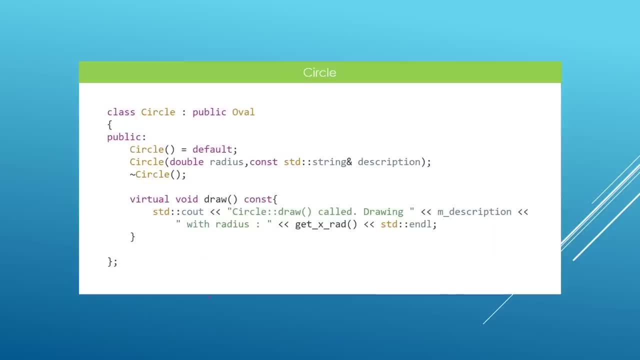 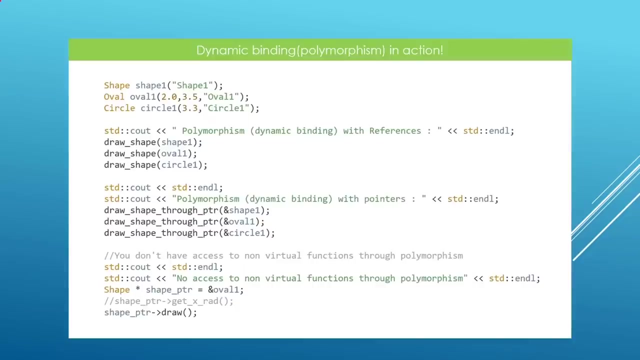 going to move in our circle class and change it to be virtual, as you see down here. this is really all we need to do from what we had in the last lecture, and this is going to be magic. let's look at what we can achieve now. we're going to set up three objects: shape, oval and circle. as you see, 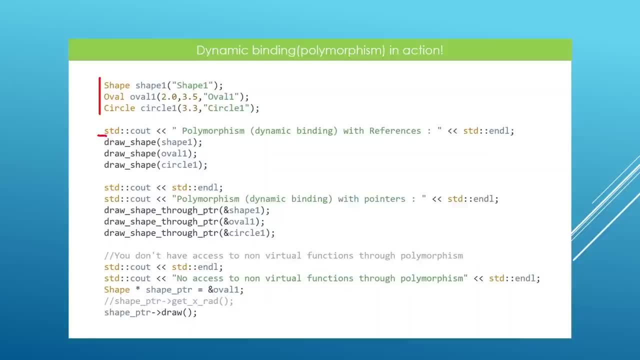 here and we're going to be calling our method, which is going to be taking references, and we're going to see that we get to the correct, most specific method called. so let's go ahead and, for example, here we will call the shape draw down, here we will call the oval draw method, because we 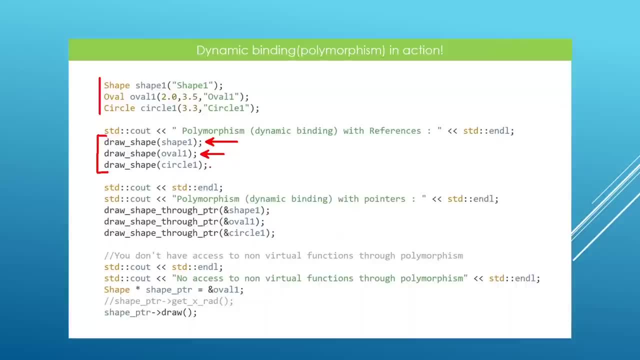 just passed in an oval object. and on the third line here we will get the circle joe method called and we will see it printed out on the console. this is really cool. this is what we want to achieve. if we want to call our methods that take pointers, we can do that. and on the first line here we will. 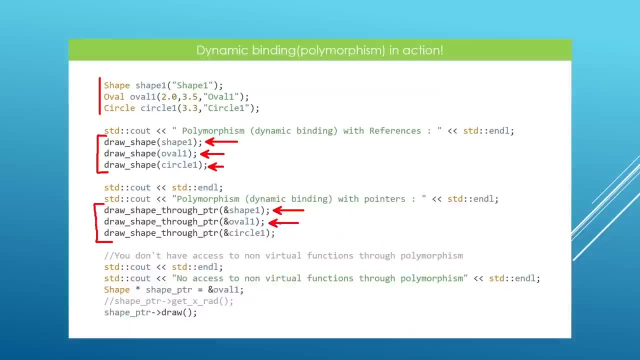 call shape draw. on the second line here we will call over draw, and on the third line, here we will call circle draw. this is what we want to achieve. and if we happen to be setting up a row base pointer, like we do here, and store in a derived object, like this or another way to say, 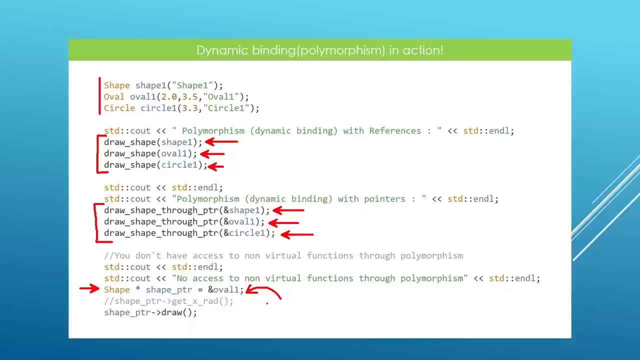 this: if we happen to be using this base pointer to manage a derived object and we call the draw method on the base pointer, the compiler is going to know that it will need to resolve this draw method dynamically. the reason is: this is a virtual method and if a method is virtual, the compiler won't do static binding like we did in. 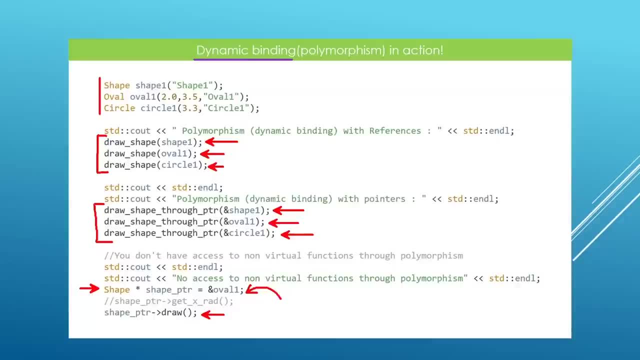 the last lecture. the compiler is going to be doing dynamic binding and with dynamic binding, the compiler is not going to look at the type of the pointer, it is going to look at the type of the actual object that the pointer is managing, and this is going to give us the behavior that we 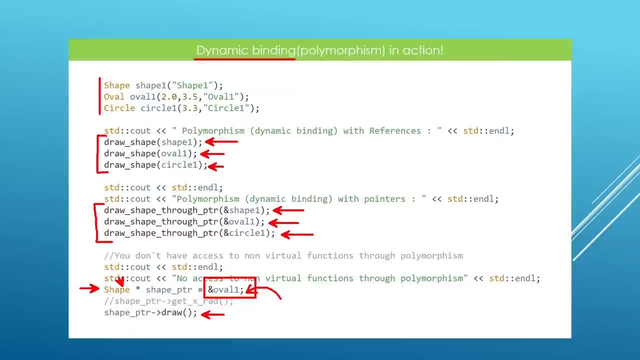 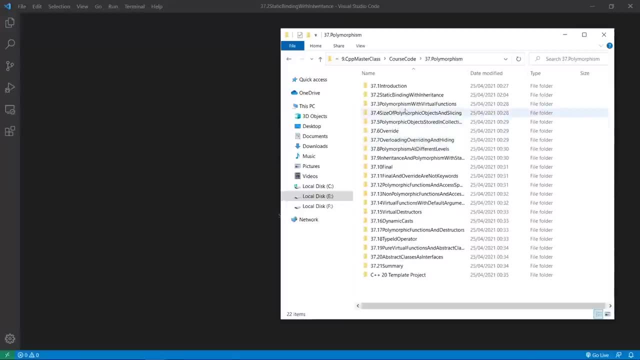 wanted, starting from the last lecture. okay, now that you know this, we're going to head over to visual studio code and play with this a little more. here we are in our working folder. the current project is polymorphism with virtual functions. we are going to be reusing the code from the last. 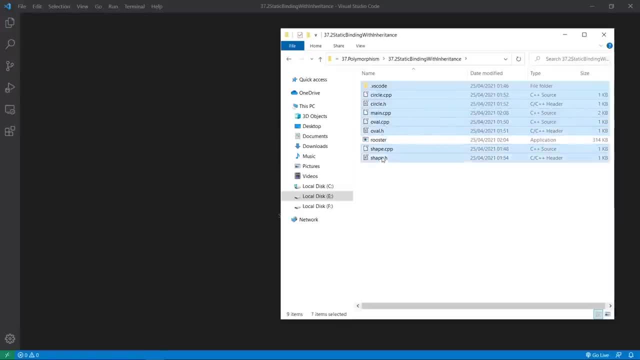 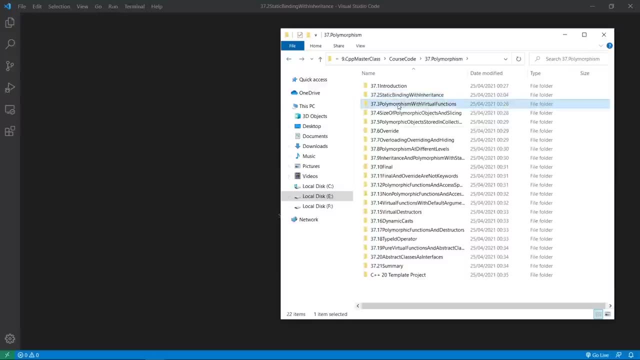 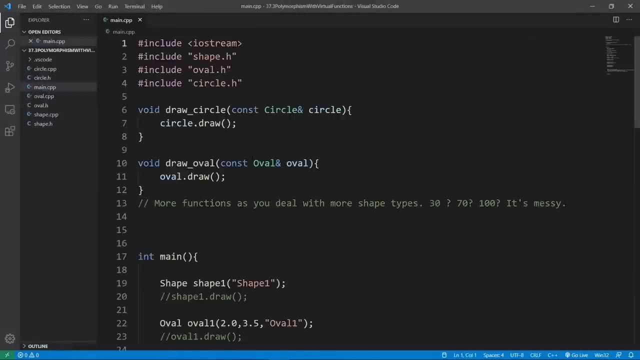 lecture, because that's going to give us everything we want. we will leave out the binary file here, which is rooster, and we're going to copy everything we want. we're going to put that in the current project and we're going to open this in visual studio code. we are going to have our main 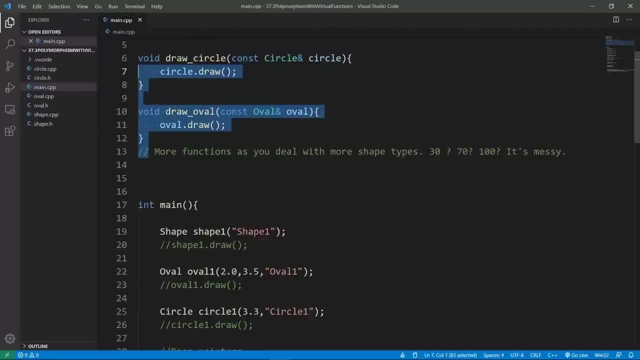 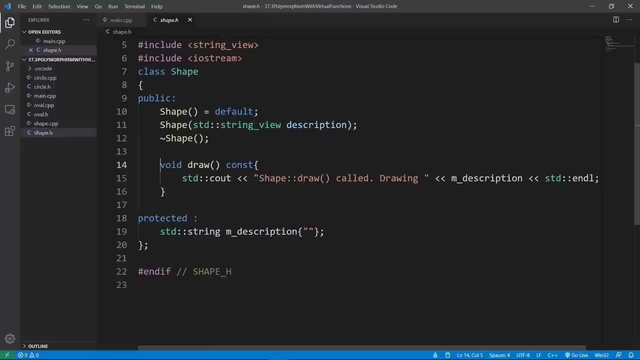 cpp file with a bunch of methods here and we will just need to modify this a little bit to achieve dynamic binding, as we saw in the slides. all we need to do is to mark all these draw methods as virtual. so we're going to say virtual void. draw in the shape class, we're going to go in the oval. 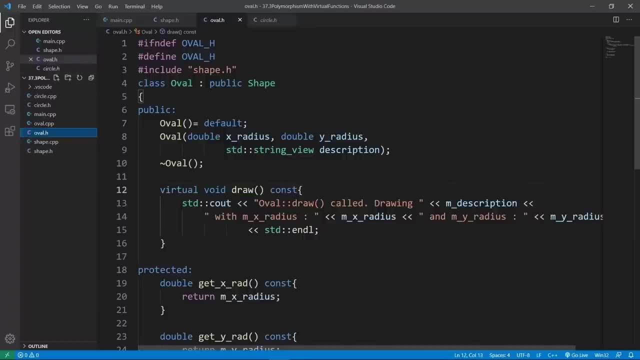 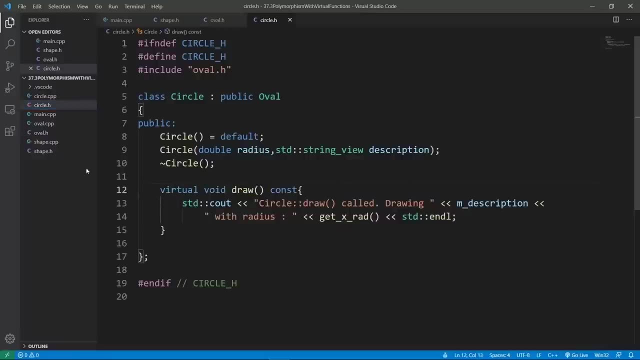 class and do that, we're going to mark our method as virtual. and we are going to go in our circle class and mark our draw method as virtual. let's do that. and the moment we do this, we're going to get dynamic binding behavior in our inheritance hierarchy here and this is really cool. so let's go back and try to play with what we had. 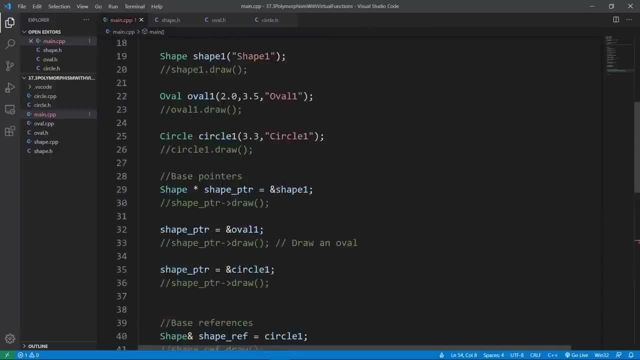 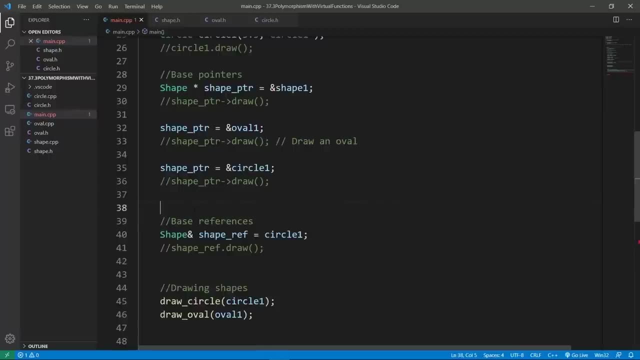 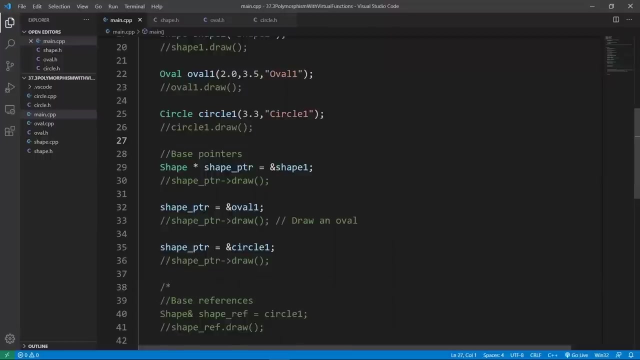 before. i am going to comment out everything we had, and we're going to be doing things in step here. let's go through the code that uses base pointers, because that's where we started out from in the last lecture and we are going to mark that here. let's put in some space to make it easy to follow. so we are going to uncomment the 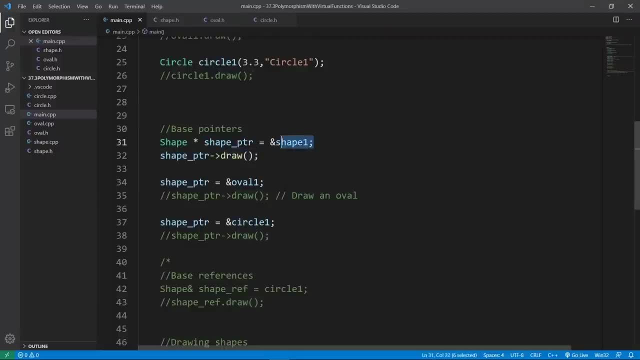 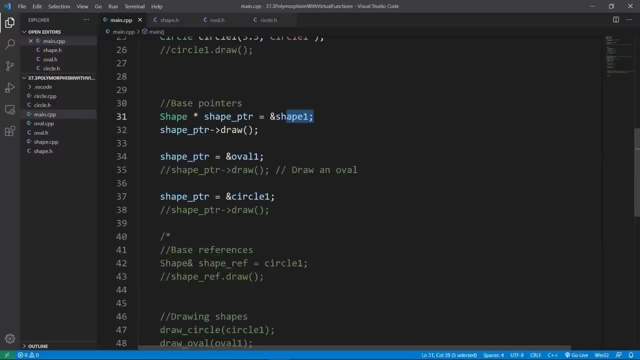 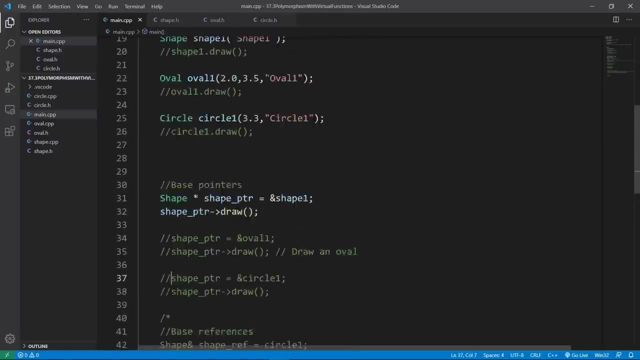 line here that calls the draw method when we have a shape object stored in our base pointer or when we are using a base pointer to manage a shape object. here we can also comment out all these lines, because we don't want this to do anything and let's see: yes, this is what we want, we are. 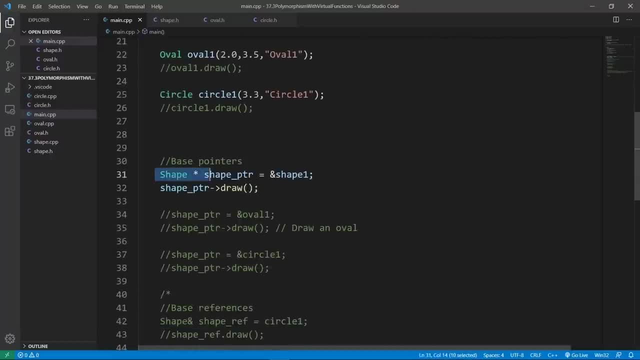 setting up our shapes and we are using a base pointer to manage an actual shape object and if we call the draw method, we expect this to call shape draw and this is what we're going to get. let's build our program. we're going to pass this through gcc, our 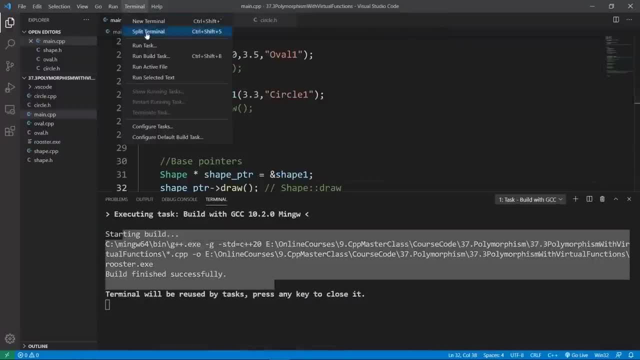 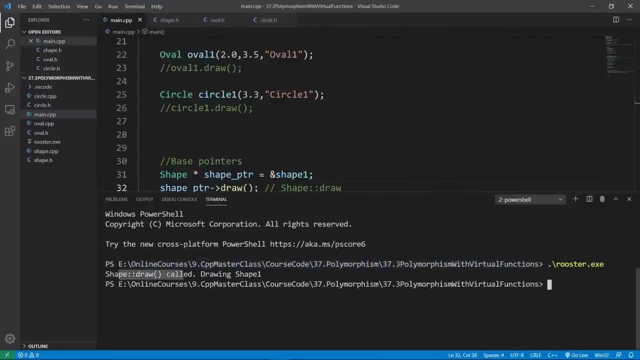 favorite compiler. the build is going to be good. we can bring up a powershell window we can use to play with us. if we call rooster, we're going to see that shape draw is called and we are drawing shape one. now, if we change this to manage an actual oval object, we can do that. we can do that. 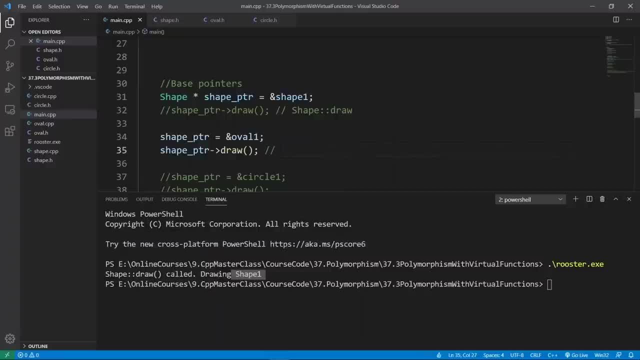 through this line here and we expect this to call overdraw. and because the draw method is now virtual, this will use dynamic binding. again, with dynamic binding, we are telling the compiler: don't look at the type of the base pointer, look at the type of the actual object that the pointer is managing and the 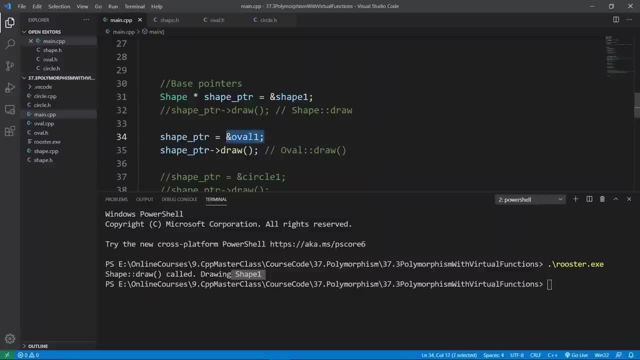 compiler is going to see that this object is a novel object and it will call the oval version of the draw method here, and this is really cool. this is what we want. let's run the task to build with gcc again. the world is going to be good, as you see here we. 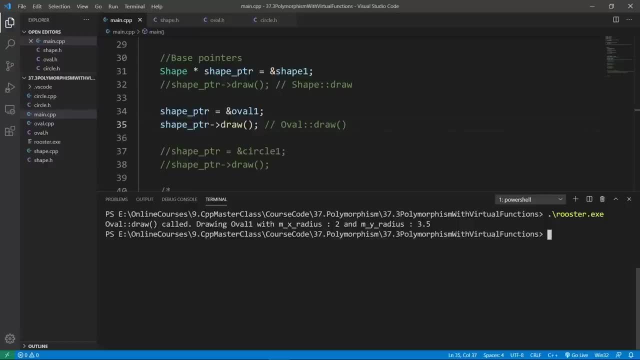 can clear and if we run booster- look at this over joe calls and we are going to be drawing our oval object and this is the data we have inside- we can use this radius data to draw this on the screen. if that's what we are after in our c plus plus program- and this is really cool- we can even use. 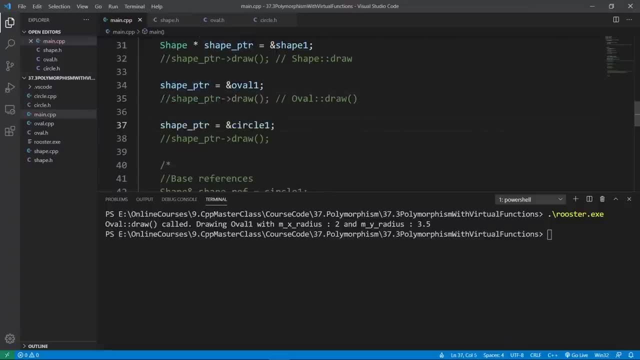 our base pointer to manage a circle object. we can do that. and if we do that and call the joe method, because this joe method is now virtual, the compiler will note that it doesn't need to look at the type of the pointer that we are using to manage our object. the compiler is going to look. 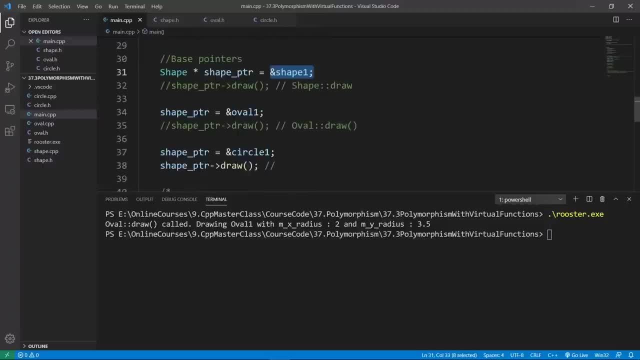 at the type of the actual object that the base pointer is managing, and in this case it happens to be a circle object. so here we will call circle draw and this is going to draw our circle on the screen, and this is really going to be super cool. so let's. 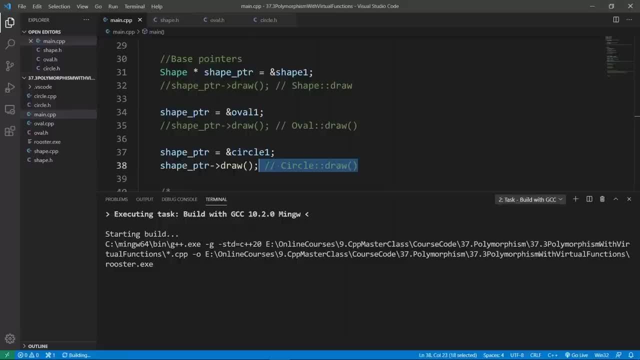 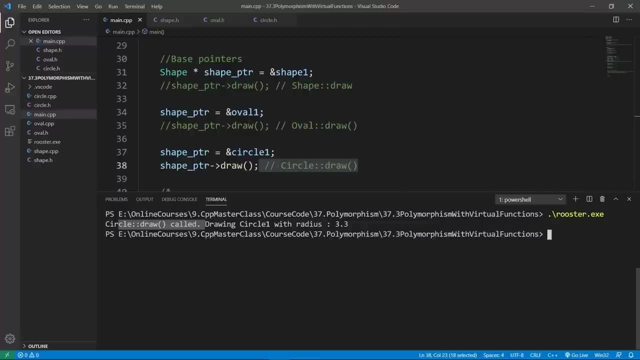 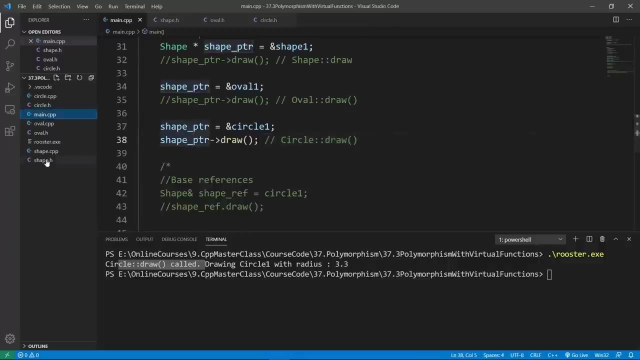 pass this through gcc and we're going to see this in action. the build is going to be good. we can clear and run rooster, and you see that we are drawing a circle, and this is really cool. and just using virtual functions we can really achieve powerful features, and you see that. 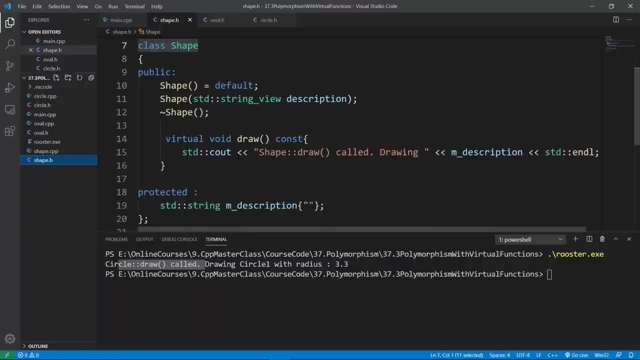 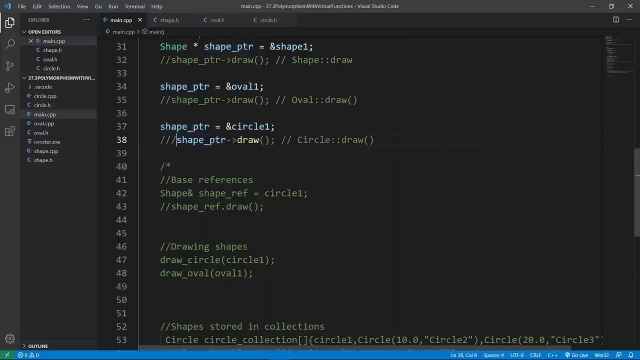 this wasn't really hard to achieve. all we had to do was to mark our inherited method as virtual, and this is going to tell the compiler to do dynamic binding, and this is going to be super cool. let's see that we can also achieve the same thing using base references. i am not going to run. 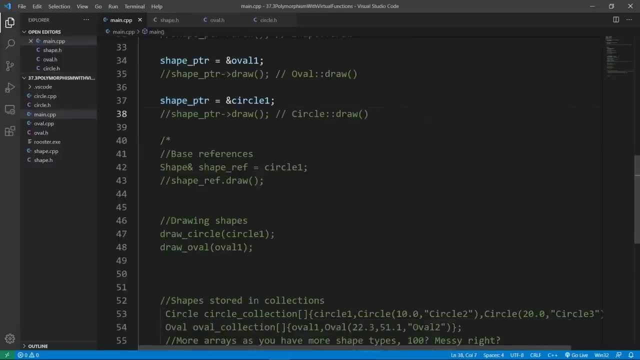 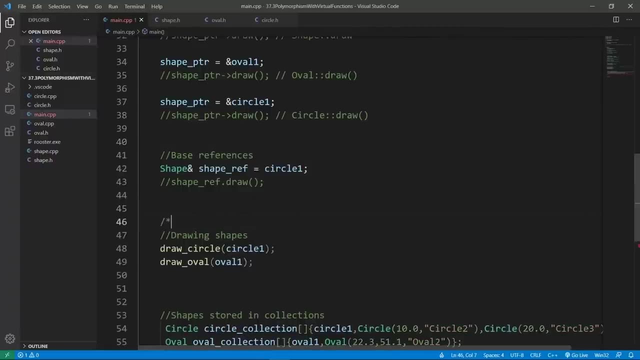 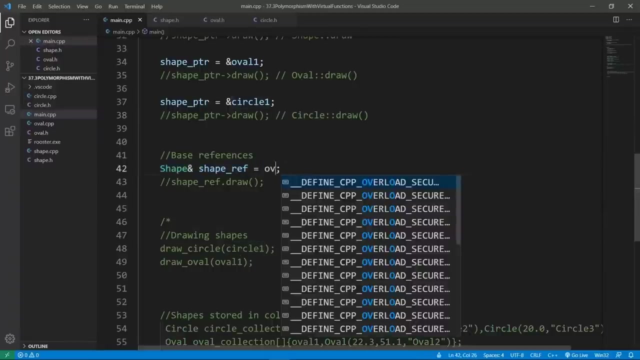 the code where we are using a base reference. i am not going to be running the code where we are using a base reference to manage a base object, because that's going to be really boring. but what we can do is put in an awful object. for example, you can say over one and say shape ref and call the draw method again. 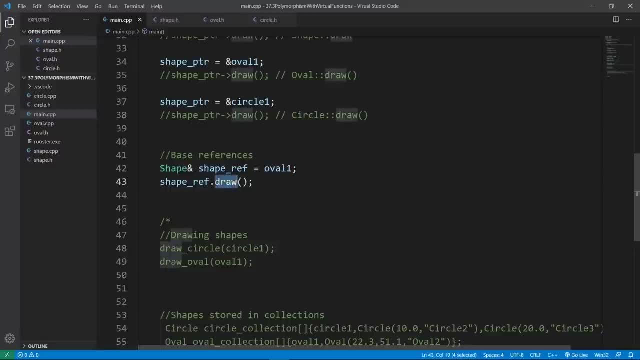 this is dynamic binding because the draw method is virtual. so the compiler is not going to look at the type of the reference to decide which version of the draw method to call. it is going to look at the actual object that this reference is managing and it is going to. 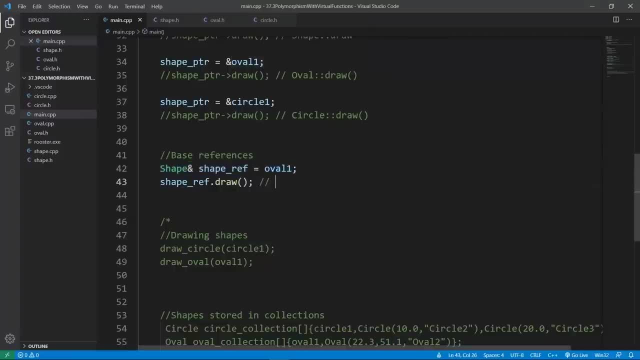 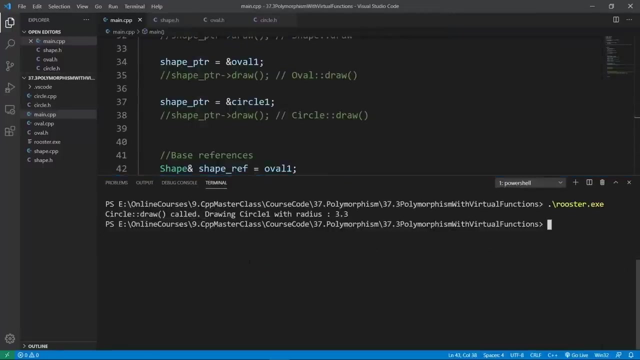 see that the type of the object is awful. so c plus plus is going to call the oval version of the draw method. that's what we're going to get if we run this program here. let's build and see this. we're going to pass this through gcc. the build should be good as we see. here we are going. 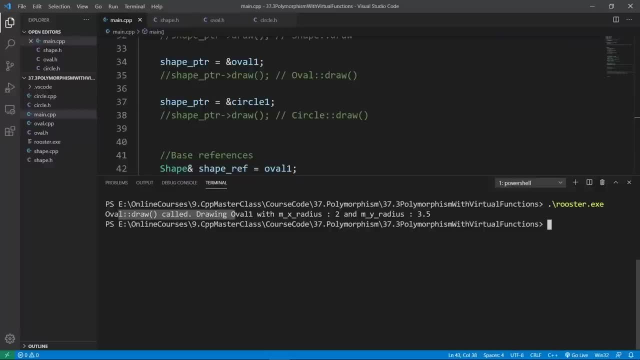 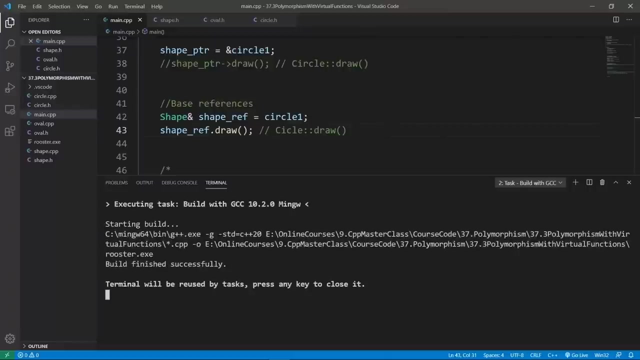 to clear and run rooster. you see, we are drawing oval. if we happen to be using this to manage our circle object, let's do that. we will see that we will get the circle method called. okay, let's bolt and we're going to pass this through gcc to do that. the board is going to be good, we can clear. 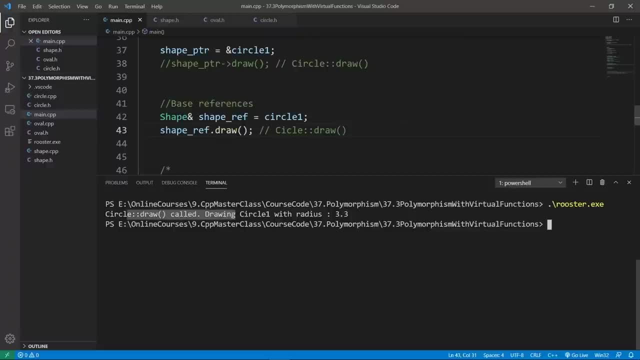 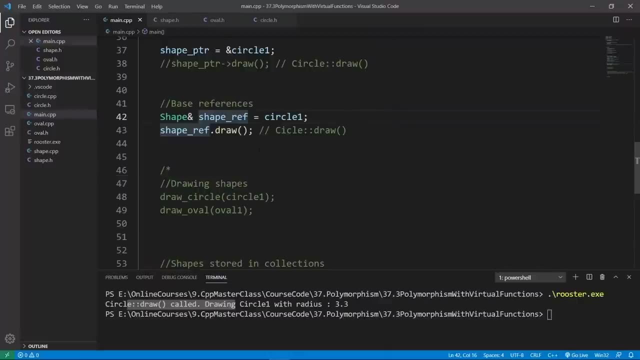 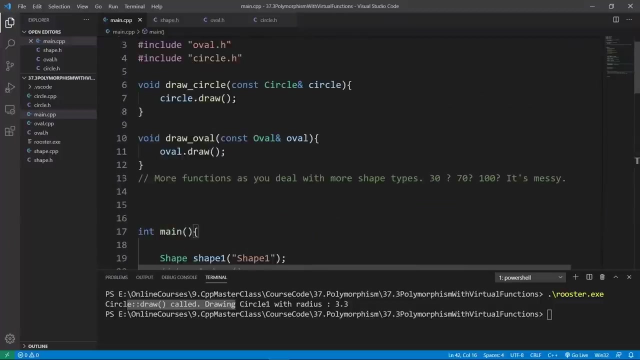 and run rooster. you see that we are drawing a circle because our base pointer is now managing a circle object. now, because we are using dynamic binding, or late binding, as some people call it, we can really do all kinds of crazy things. the first thing we can achieve is set up one single method. 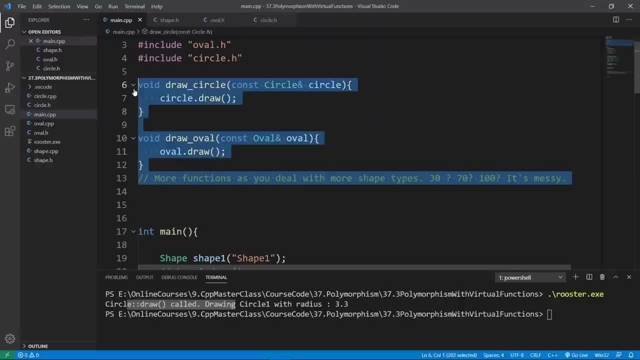 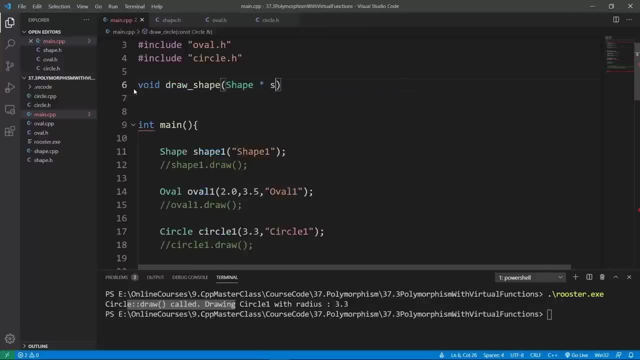 which is really going to draw any kind of shape we throw at it. so let's do something like this: we're going to say void and we're going to say draw shape, and it is going to take a shape, point here. let's say s and the only thing we're going to do in this function is say s- draw. this is going. 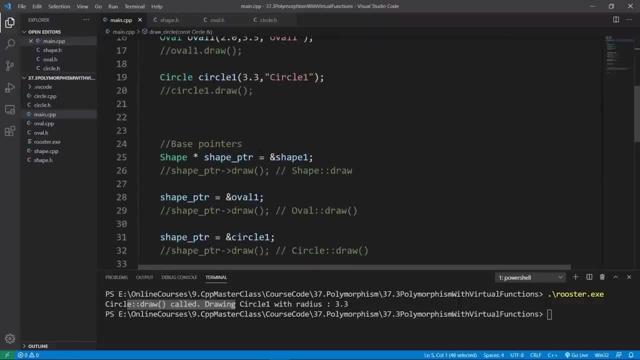 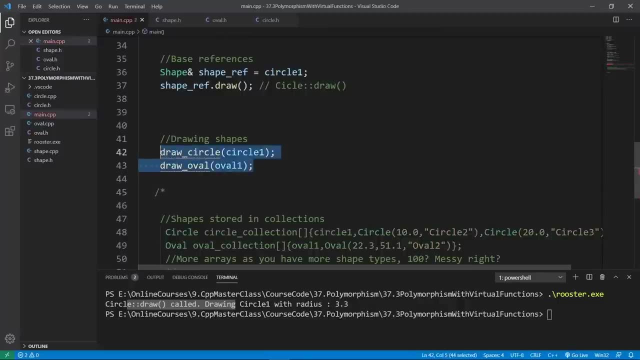 to call the draw method on whatever parameter that we pass in here and watch this. if we go down here and and comment this section on drawing shapes, if we say draw and pass in a circle, for example, or let's pass an oval and do this one level and do this level by level, we're going to pass in oval 1. 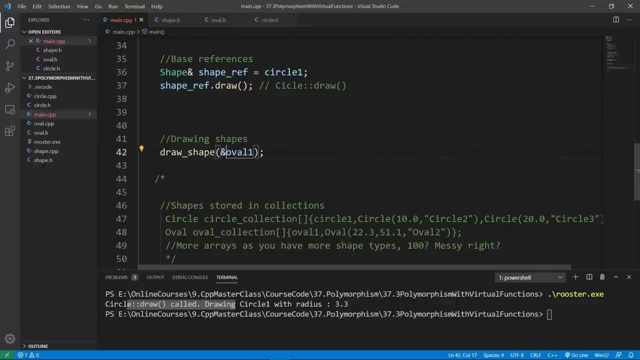 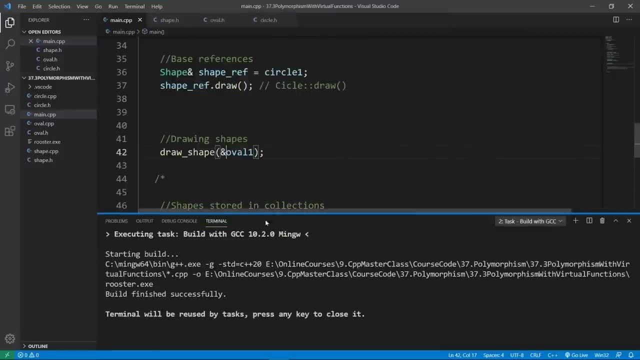 and we should pass an address because this is taking a pointer. let's so, let's do this. and if we build and run this program, let's see what happens here. we're going to build with gcc. the world is going to be good, as you see here, if we clear and run rooster. 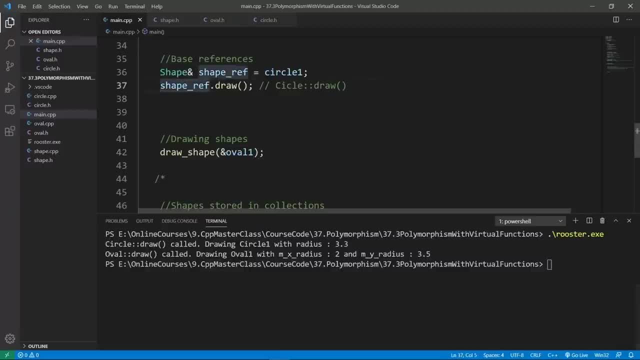 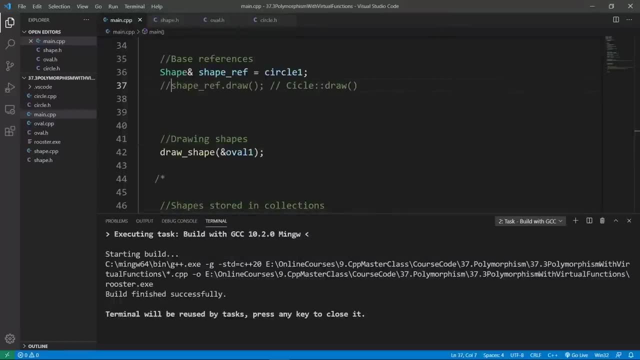 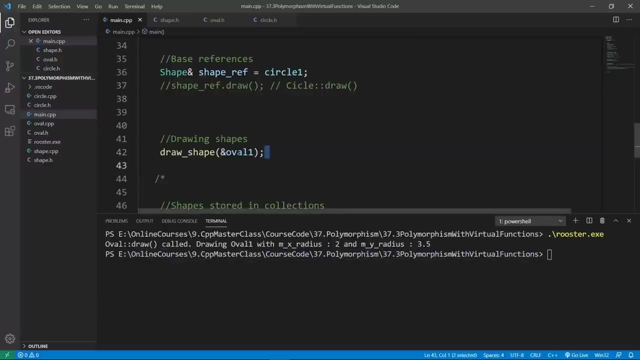 you see- and let's take out this thing using base references here, because this is just going to confuse us- we're going to build again and i use gcc for this. the world is going to be good. we can clear and run rooster. you see oval draw, because we are passing in a novel object. if we pass in, 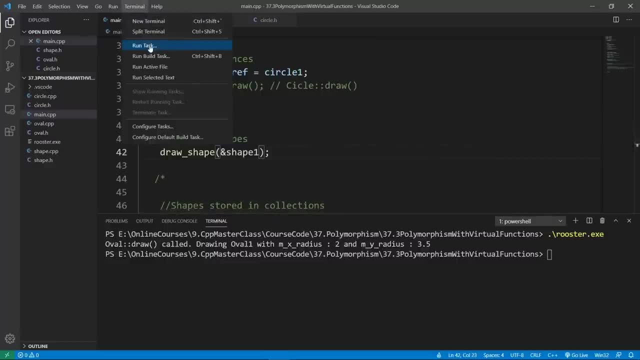 our shape. let's say shape one, for example. we're going to build, the build is going to be good, as you see here, if we clear and run rooster, we're going to see shape draw if we pass in circle, let's do that and both again, we're going to build with gcc, we're going to clear and run rooster. 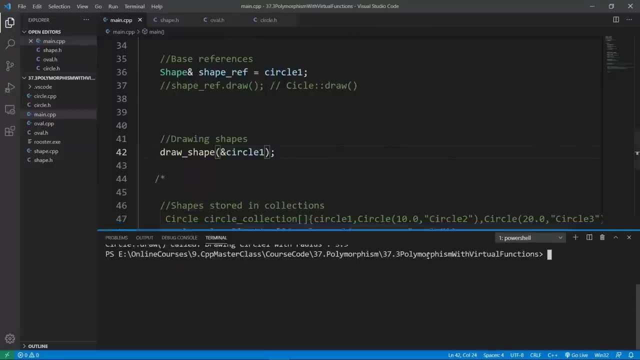 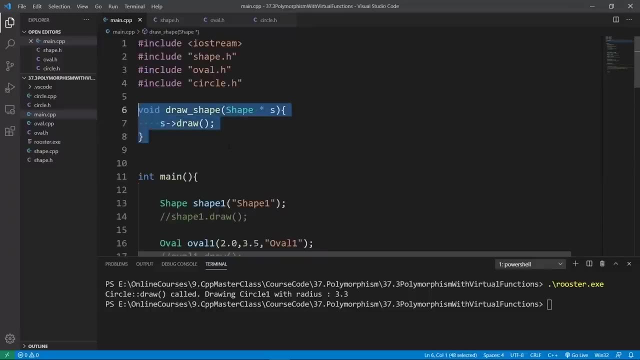 you're going to see that circle draw is called, and this is really cool. we can only use a single method and this method is going to take any shape we throw at it and it is going to draw it. if we happen to get the correct shape in our collection, we can just, for example, loop through a collection. 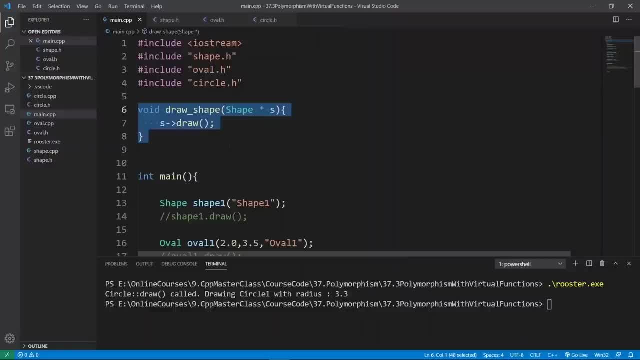 containing those shapes, and if we call the draw method on any shape we store in our collection, we're going to get the correct shape drawn and this is super cool. this is really powerful and i hope you are excited to be able to achieve this in c plus plus. now we can also achieve the same. 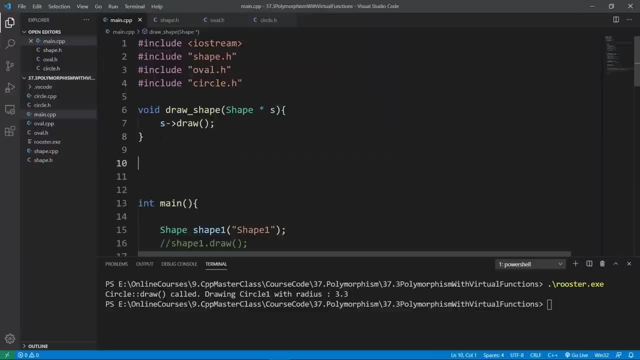 thing by using a method that takes a reference, for example. so we can say void, draw shape, let's say v1 and we're going to pass a reference. we can say cost and pass a reference, and say s? r to say shape reference. we can do that and we're going to say s joe, we're going to call the joe. 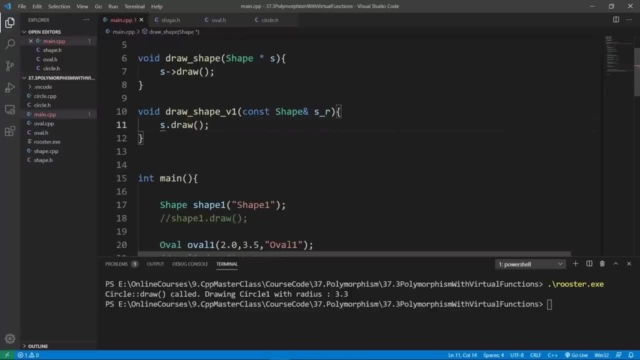 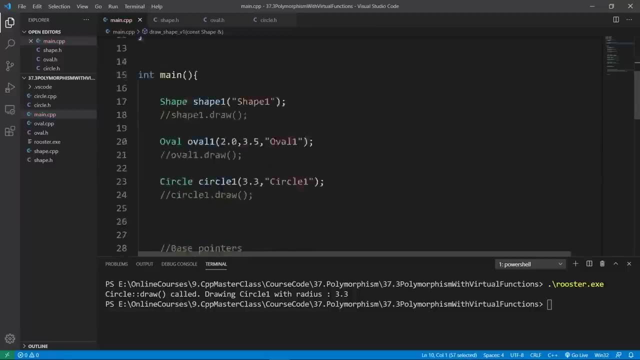 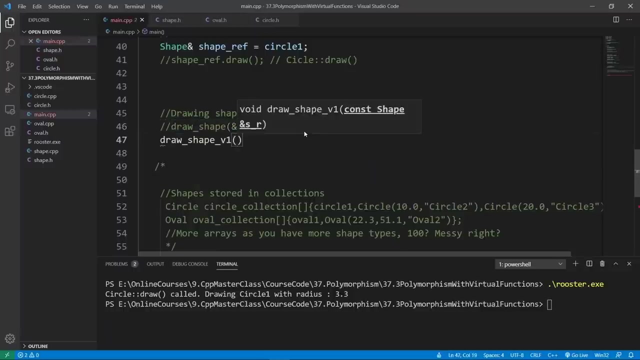 method on this reference and let's see what happens if we try this out. let's say sr. that's what we should say here, and this is going to be taken by our visual studio code editor. if we go in here and change this to say draw shape v1, we can pass it. 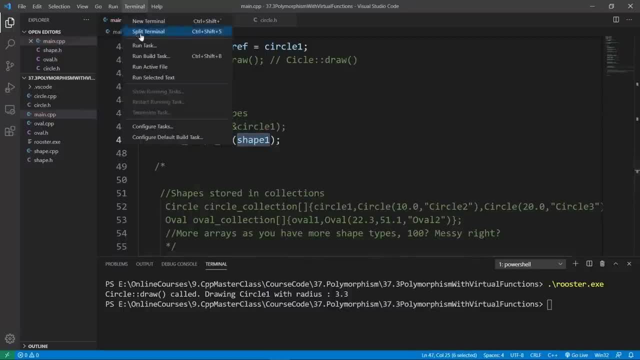 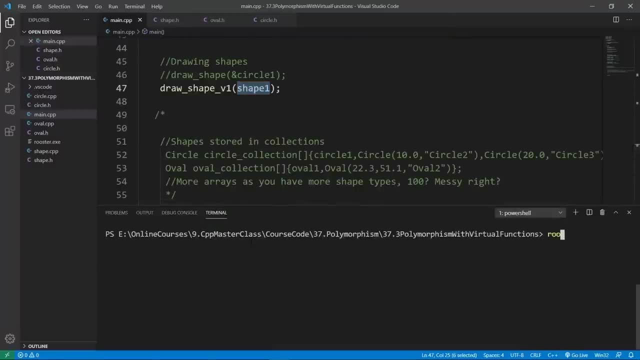 shape one. we can do that because this is taking a reference. now, if we build with gcc, we are going to see that the world is good. we can clear. let's clear: we're going to run rooster. this is going to call shape draw, because we are using a reference to manage a shape object. we can also pass in over. 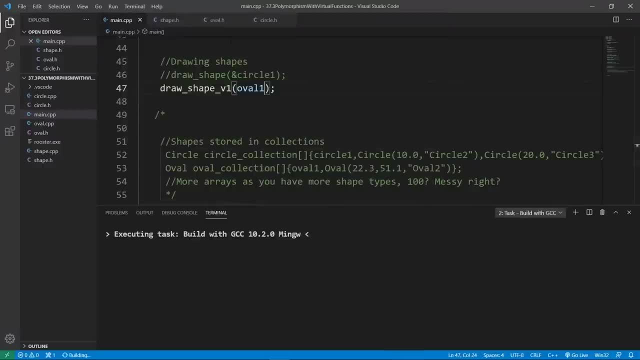 one and we're going to build again and see how this works. the build is going to be good. we can clear and run rooster. we're going to say over draw and we're going to see our information here passing our circle object and the bolt. we're going to pass this through gcc. the world is. 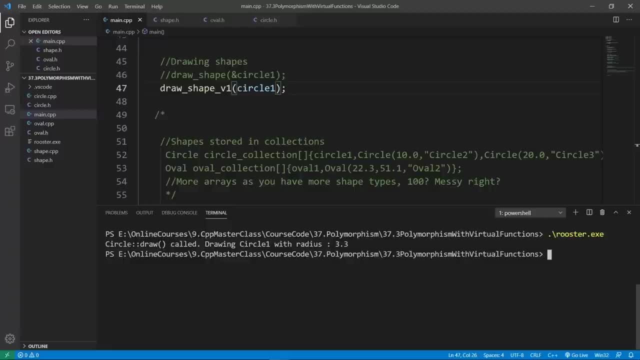 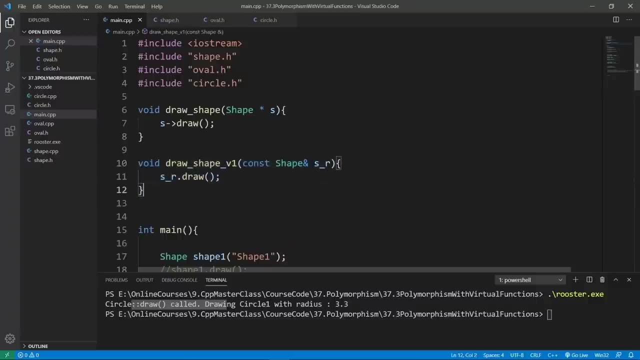 going to be good. we can clear and run rooster. this is going to draw a circle for us. this is really cool. we have one method again that is taking a parameter by reference, but we can use this method to draw any kind of shape in our inheritance hierarchy. this is going to work. 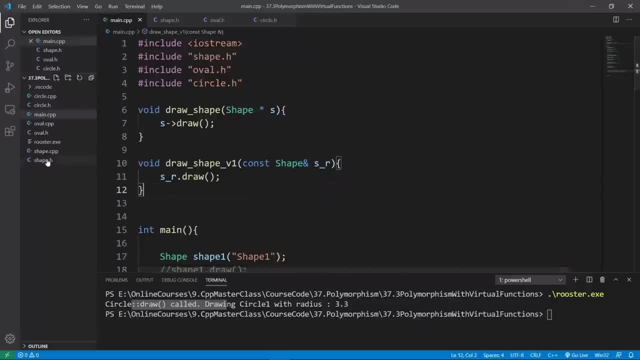 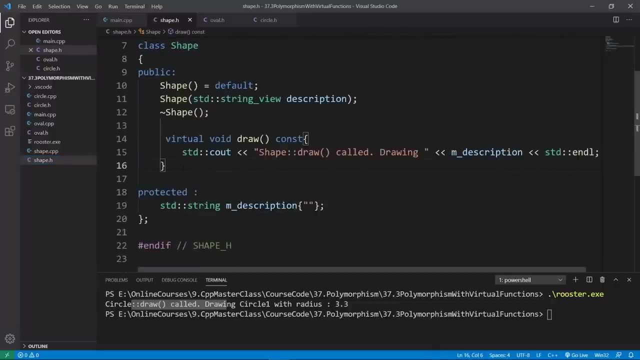 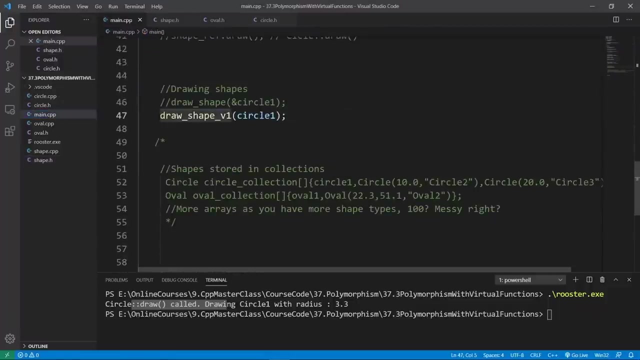 really well and it is doing dynamic binding which is powered by virtual functions we are using in our inheritance hierarchy here. you should really keep this in mind. now let's go back and see if we can even use row pointers to do stuff. i am going to comment this out and i am going to say: 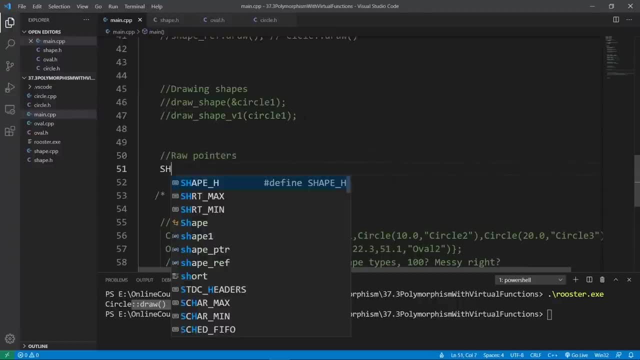 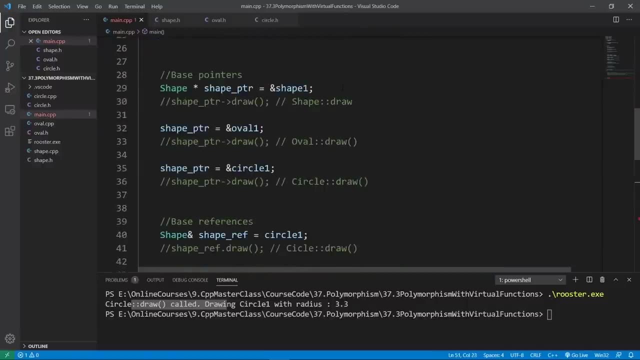 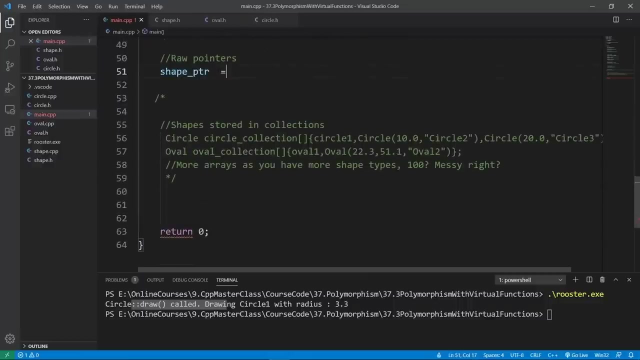 row pointers, because i want you to see something. we're going to set up a shape pointer. we're going to say shape ptr. do we have that on top here? let's see if we do. yes, we have shape ptr. so let's say we're going to pass an oval again and we're going to pass the address of over one. this is going to 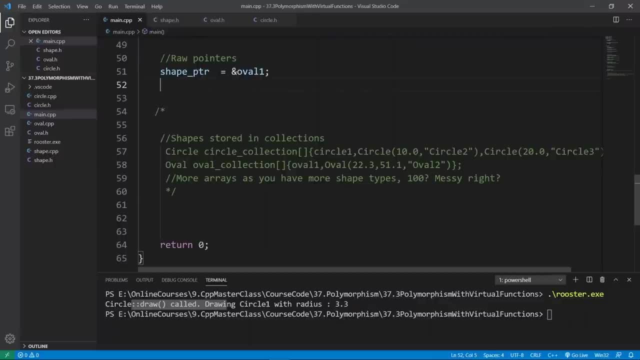 do? we can call the draw method and get it called polymorphically, or get it called using dynamic binding. we can say shape ptr and say, joe, this is going to call the correct version. but one thing i want you to see is that if a method is not polymorphic or if a method is not virtual, 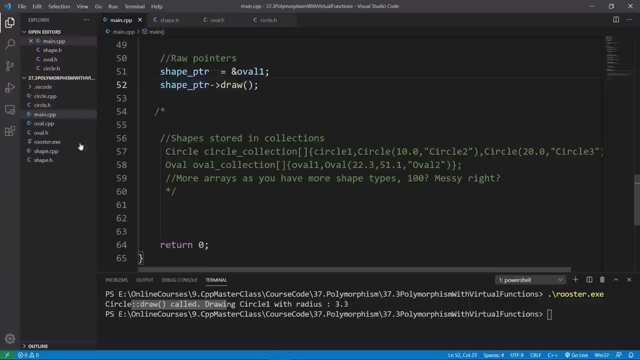 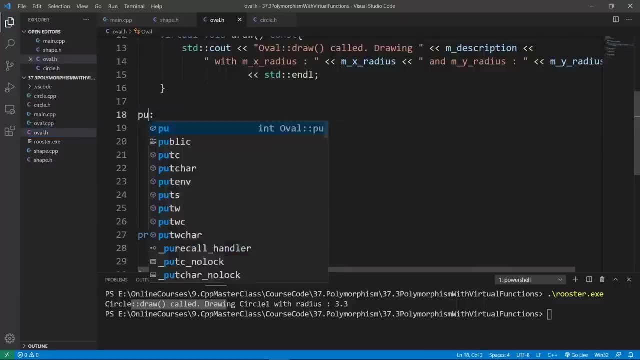 you won't get it called using polymorphics polymorphism. for example, if we go to our ovo class, we're going to see that we have a bunch of getters. let's go in and make them public so that they are callable from the outside. and if we try and get 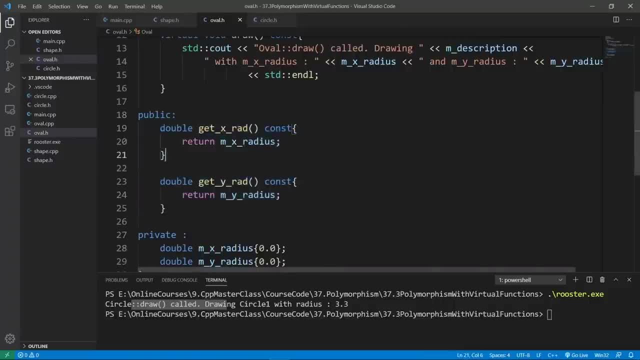 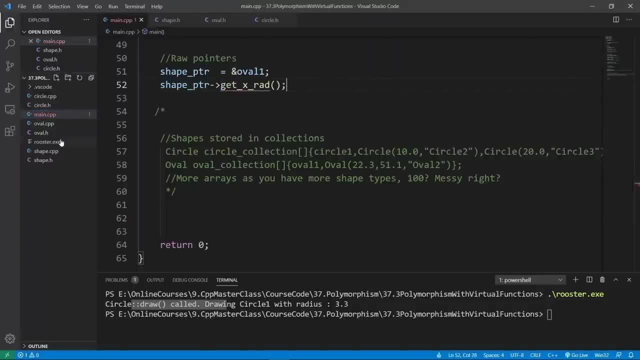 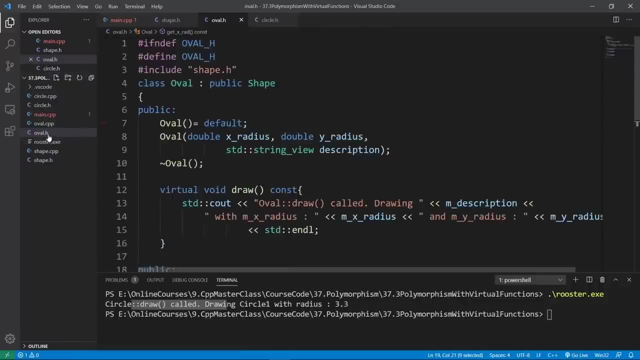 this called polymorphically or using dynamic binding. that's not going to work. let's do that. we're going to say get x rad. and the reason we might want to do something like this is because we have this method here and it is set up on our ovo class, so because we are using a base pointer. 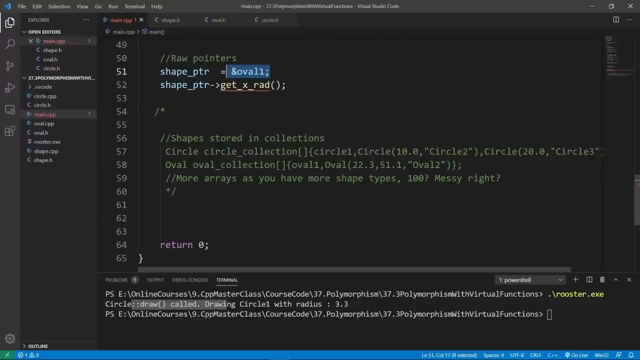 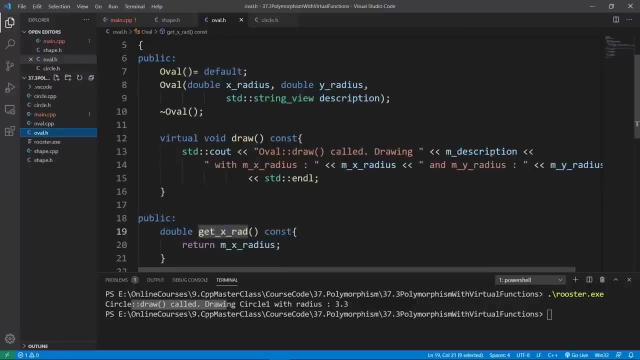 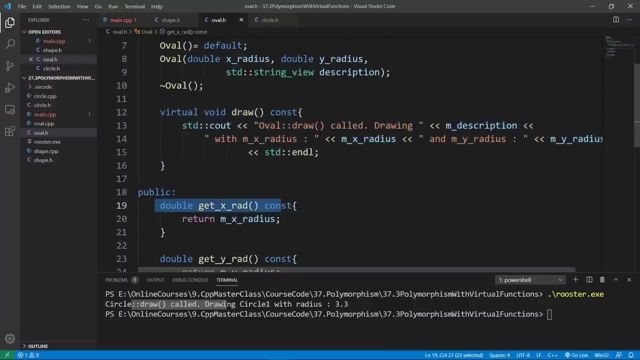 to manage a novel object. some of you might think, uh-huh, i might be able to call this method because i am able to call the joe method, which is also in the public scope of our ovo class. but that's not going to work because this method here is not virtual, dynamic, binding or polymorphism. 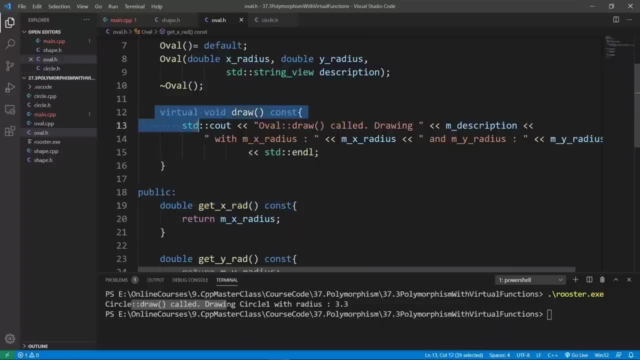 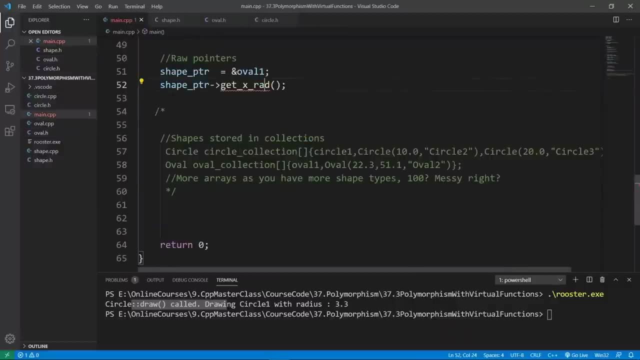 is not going to work because it's not going to work because it's not going to work because only going to work if your methods are virtual and they are set up across your inheritance hierarchy. so this is not going to work. if you try to do something like this, this is going to give you. 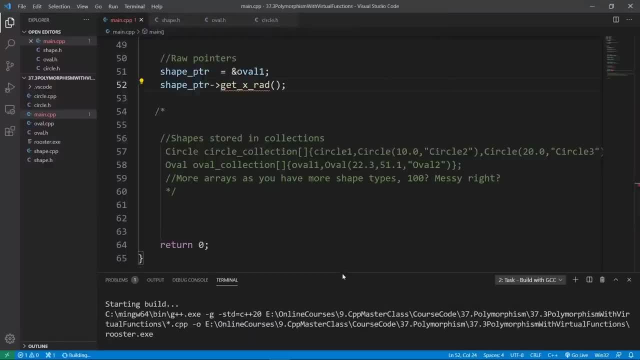 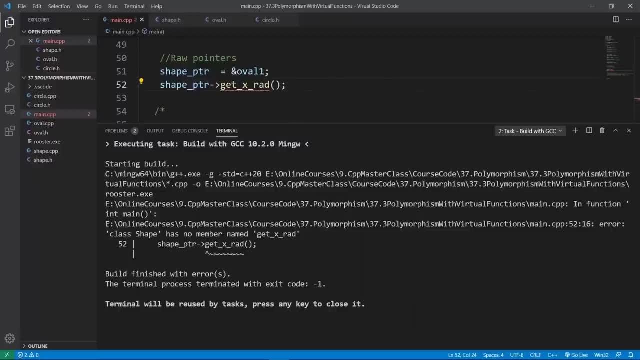 a compiler error. let's try and world and i see the compiler error and we're going to see an error that says that no such method on this object. let's go here: class shape has no. class shape has no member named. get x rad because the method is not virtual. the compiler is going to do static binding. 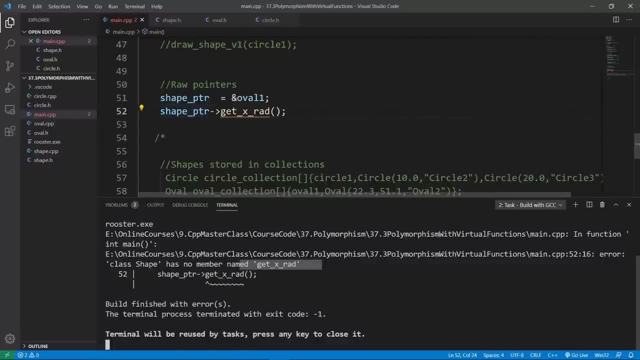 and it is going to be using the type of the pointer which is shape to resolve this method and it is going to see that in shape we don't have a method called get x rad and the compiler is going to throw this compiler error here. this is what we get. so this is not going to work and i 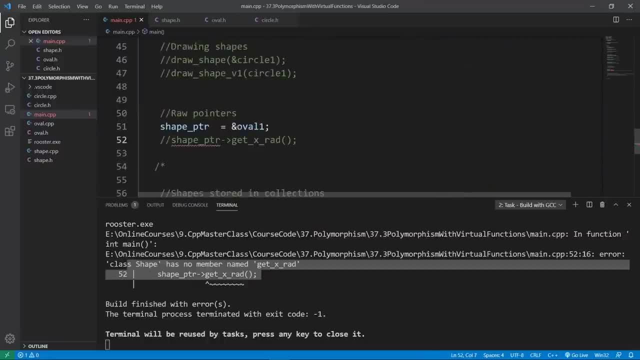 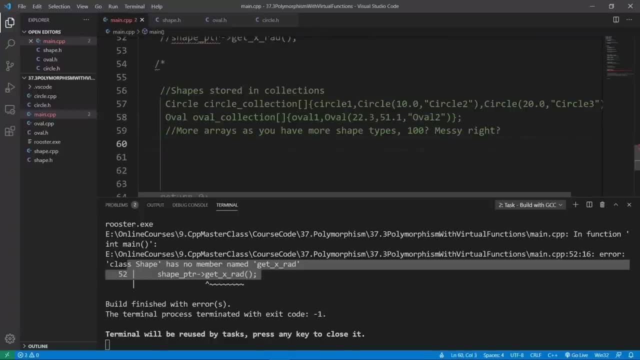 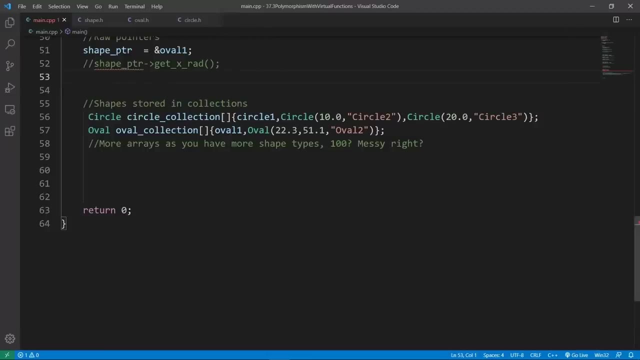 want you to be aware of this. another thing i want you to see is that because we are using the dynamic binding now, we don't need- we don't need to set up all kinds of crazy collections to take into account different shapes that we have in our c plus plus program- what we're going 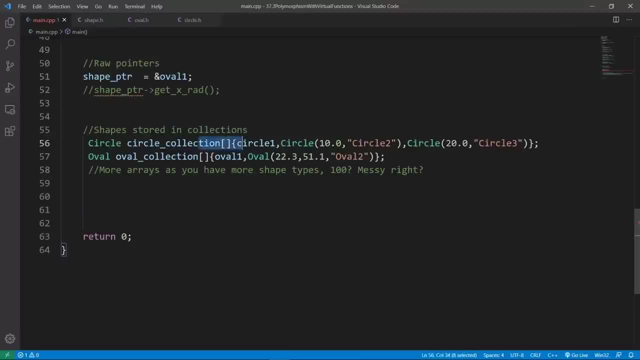 to do here is use a base pointer to manage the data that we store in our array here. so all i am going to do is remove all this dirt here, because this is really dirt. you don't want to do something like that, and we're going to use a base pointer, which is a shape pointer. 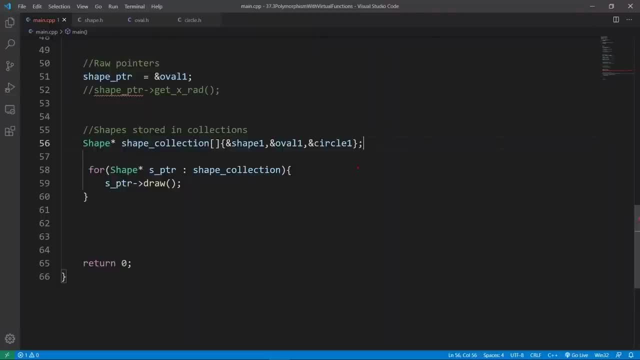 and use that to set up an array which can handle any kind of shape we have in our inheritance hierarchy. so we can store in shape objects, we can store in oval objects, we can store in circle objects and if we look like we do here, we're going to get the correct method called and this is going. 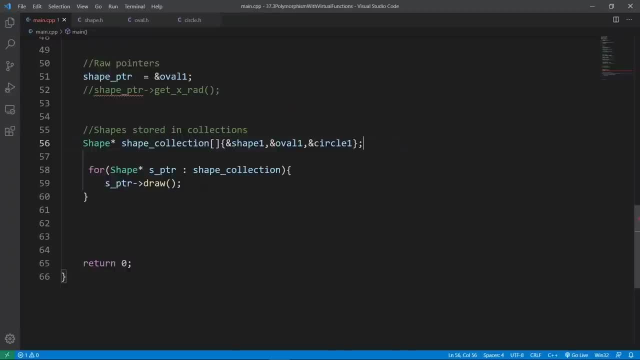 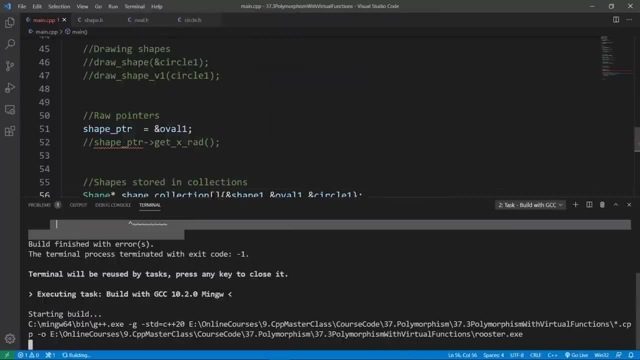 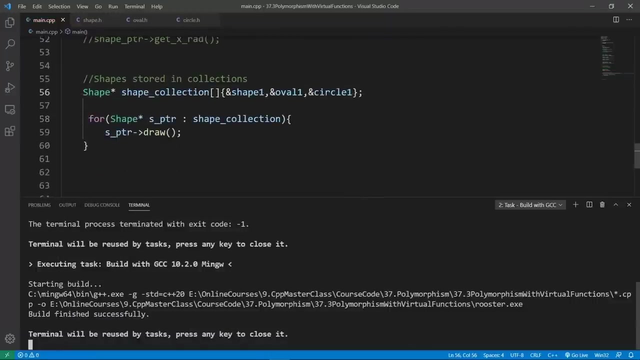 to be super cool, so let's try and run this program. we're going to pass this through gcc. why do we have the red thing here? let's build and see if it goes away. maybe this is vicious studio code having a problem with our code. the world is good, so visual studio code was playing. 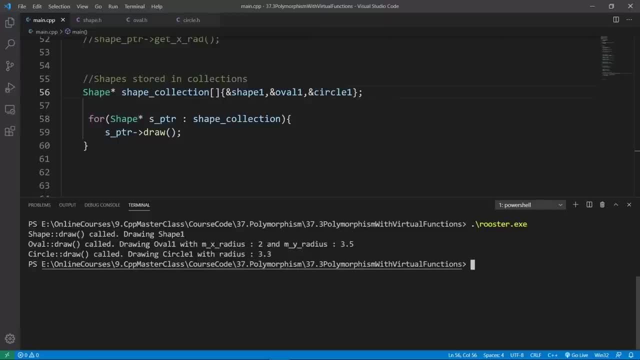 with us. we're going to clear and run roaster. you're going to see that we're going to be looping through this array here and on the first iteration we're going to call shape draw, because the first thing is a shape. on the second iteration, we're going to call over draw, because the second thing 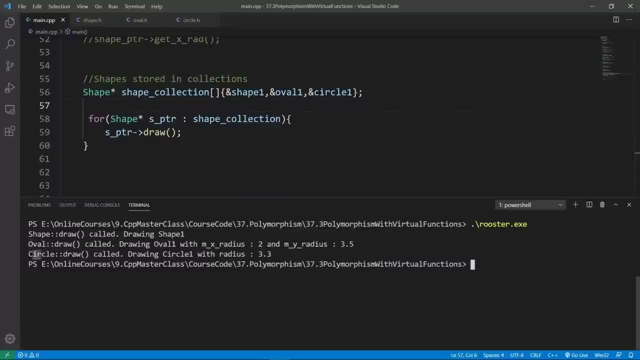 is a novel and we're going to hit the third iteration and call circle draw, because the third thing in this collection is a circle. hopefully you can see that this is going to simplify our programs a lot compared to what we were able to do in the last lecture, and this is really all i had. 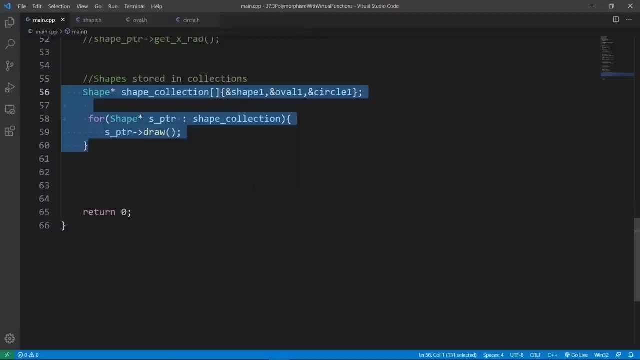 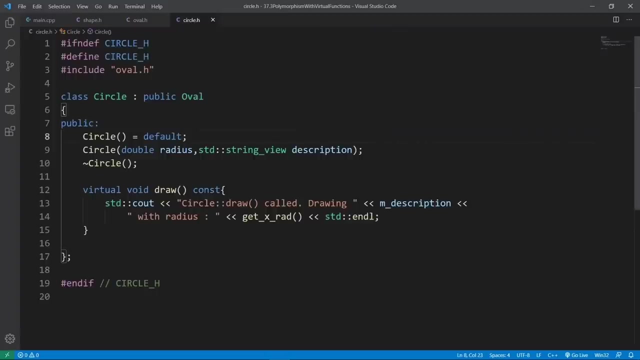 to share in this lecture, showing you that you can achieve dynamic binding, or polymorphism, or late binding as some people call it, using virtual functions in your inheritance hierarchy. again, all we had to do was mark our member functions as a virtual and the compiler is going to know that it can set up dynamic polymorphism for your types if you. 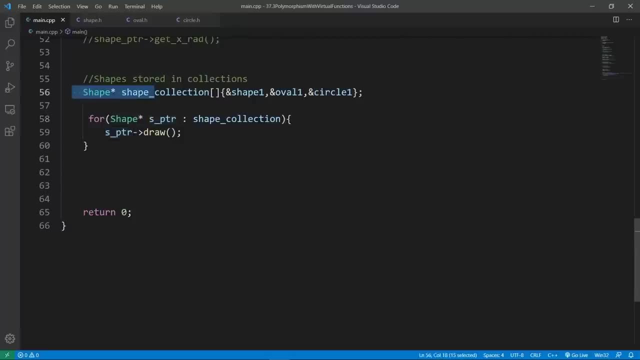 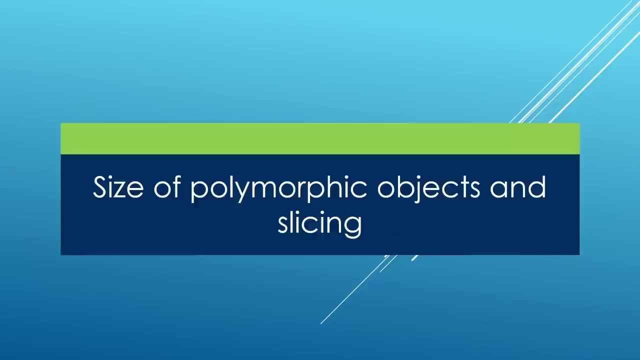 happen to be managing them using a base pointer or a base reference. we are going to stop here in this lecture. in the next one we're going to learn about slicing and the size of polymorphic objects. go ahead and finish up here and meet me there. in this lecture we're going to explore 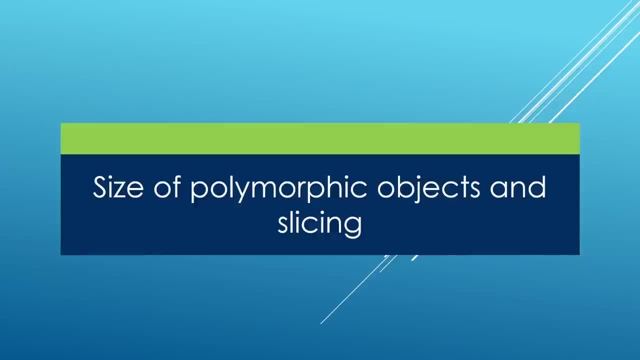 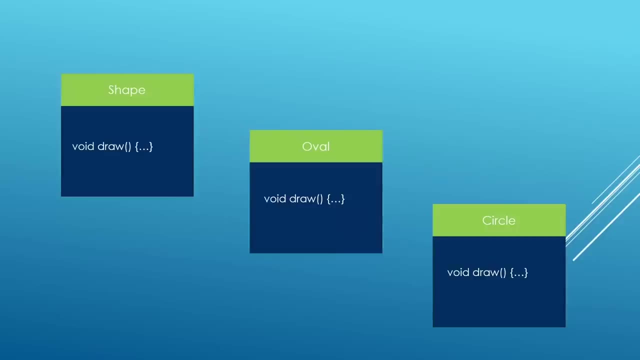 the size of polymorphic objects or objects that use dynamic binding, and we're going to learn about the concept of slicing. if you happen to assign a derived object to a base object. we're going to see how this works out. in the last two lectures we saw that we could achieve static binding. 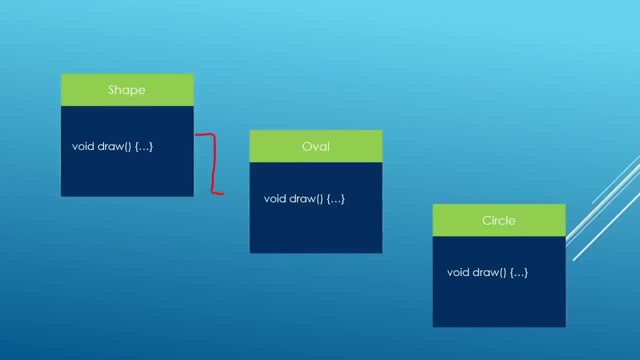 using a setup like this, we can set up an inheritance hierarchy and we're going to have oval derived or inherit from shape and we're going to have circle inherit or derive from over here, and our methods are going to be row, they are not going to be virtual on anything, and this is going to do. 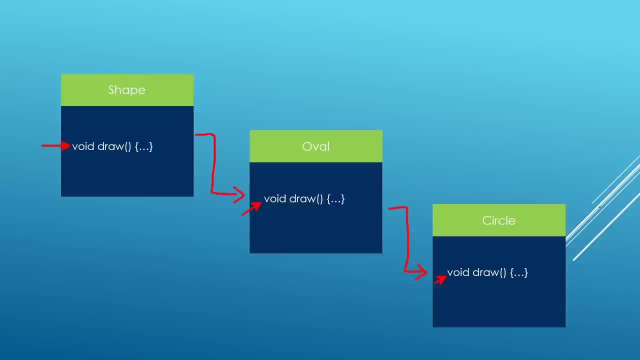 static binding. if you happen to manage a derived object through a base pointer or reference, you want to get dynamic calls, you will get static binding and the compiler will use the base pointer or base reference to decide which draw method to call on your object. we also saw that we could 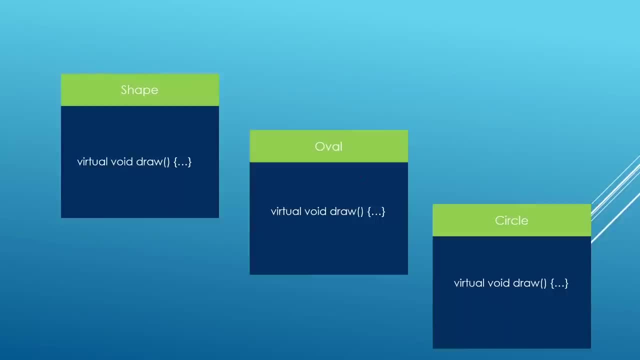 achieve dynamic binding using virtual functions, and all we needed to do was to mark our methods as virtual in our inheritance hierarchy here, and this would give us polymorphism or dynamic binding. but one thing you should know is that dynamic binding is not free. you're going to be paying. 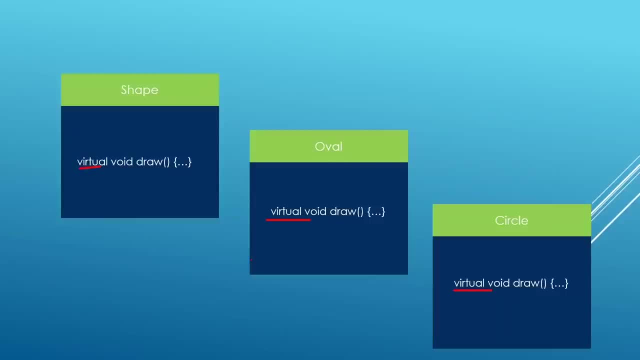 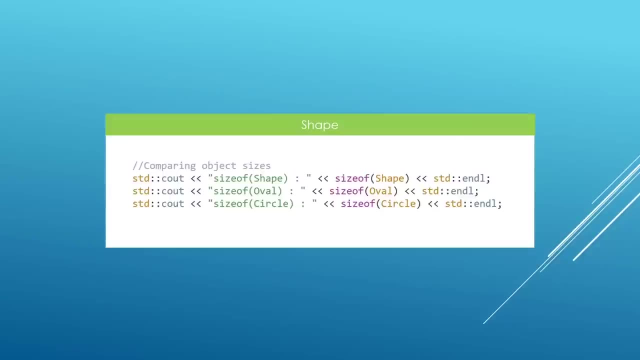 in terms of memory, to get all these cool things we saw in the last lecture, and we're going to be proving that in this lecture. what we're going to be doing is basically set up our inheritance hierarchy, and we are going to set that up in such a way that it is 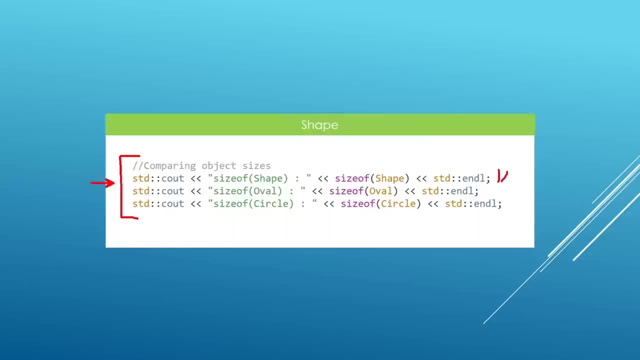 going to be using static binding. we're going to see the sizes we get printed out here and we're going to use dynamic binding and compare the sizes and the constatation is going to be that with dynamic binding your objects are going to be much larger because your c plus plus program. 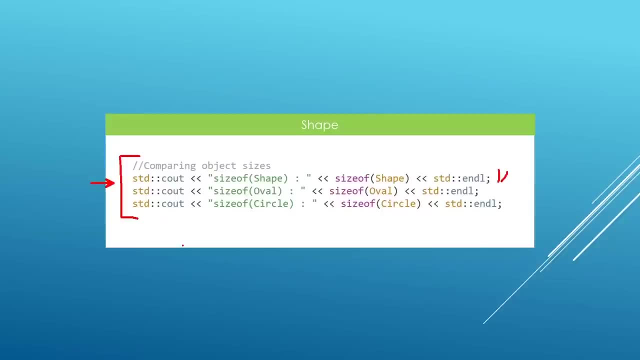 will need to keep track of the information that allows it to resolve function calls dynamically, and that information is stored in what we call virtual tables. but i am not going to go into that here because it is really out of scope of a course like this. but i want you to be aware of this: if you use dynamic, if you use dynamic binding, your objects are going. 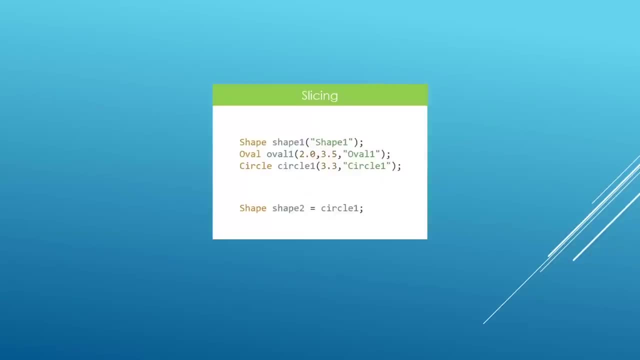 to be much larger. okay, the first thing i want to bring your attention to is object slicing, and we're going to look at a simple example here. we have our objects, we have shape object, we have an oval object and we have a circle object, and down here we want to assign. 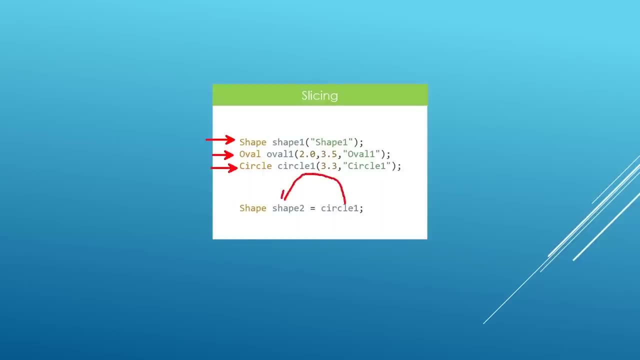 our circle object to a shape object. now, notice that here we are not using a pointer or a reference. these are just row objects that we are assigning to each other, and what the compiler is basically going to do: it's going to notice that a circle has a shape, port into it and it is going to strip off. 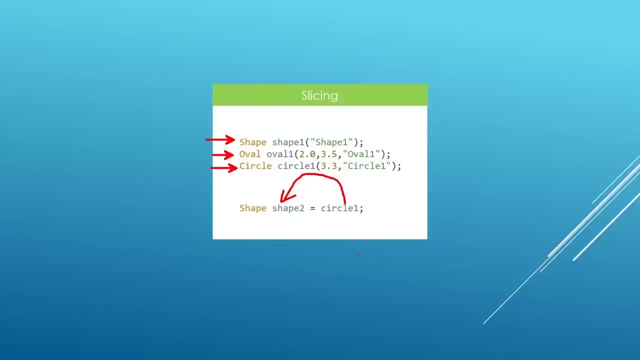 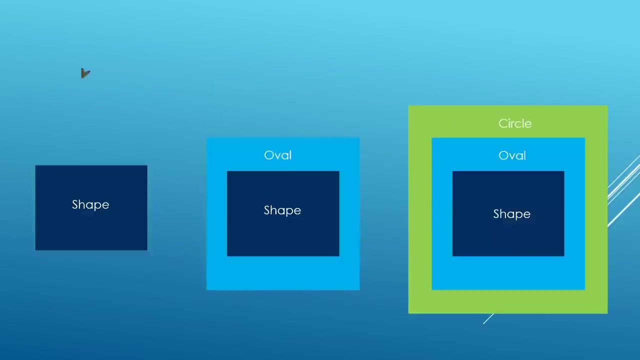 layers, or in other words, it is going to strip off the circle layer, it is going to strip off the oval layer and it is going to leave in the shape part, and that's what it is going to assign to our shape object here. let's visualize this. our shape class looks like what we have here on the left. 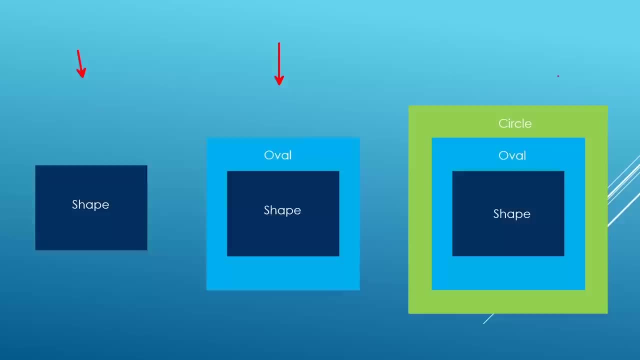 our oval class has a shape part into it and our circle is going to have an over part into it and that over part is going to have a shape part of it, and this is the setup that we have here now. if we do our assignment, we're going to do something like this. 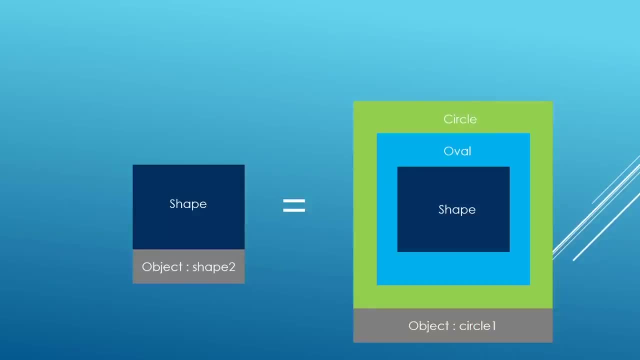 the compiler is going to see that we are already assigning a circle to a shape, and the compiler is going to notice that what we have on the left is just a shape and we don't have enough space to store information about oval and the circle here. so what the compiler is going to do, it is: 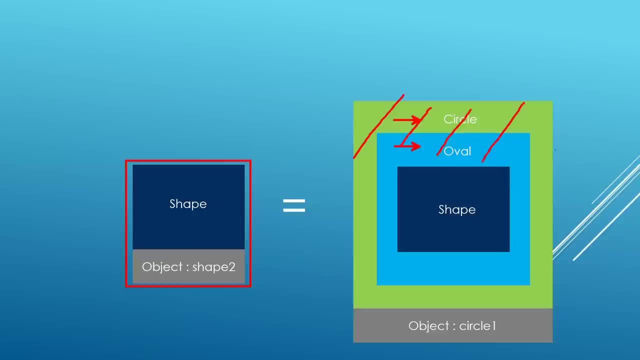 going to strip off all these things that we don't really need and it is going to leave in only the shape part that we can assign on what we have to the left. so it is going to strip off all these things and we are going to be left with something like this, and then what we have on the right is: 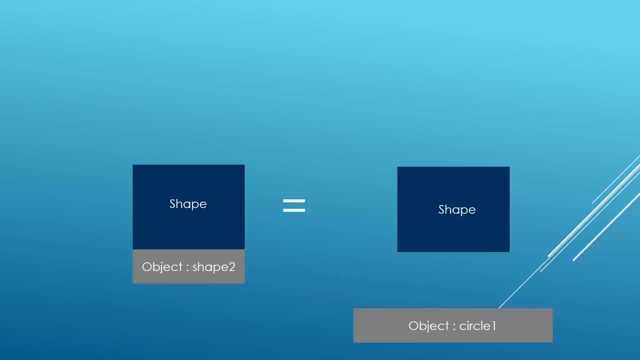 going to be assigned on the left and we will have our data stored in our shape to object and if we try to use it, that's what you're going to get in memory. so this is referred to as slicer. again, the compiler is going to notice that it doesn't really have enough space on the left to 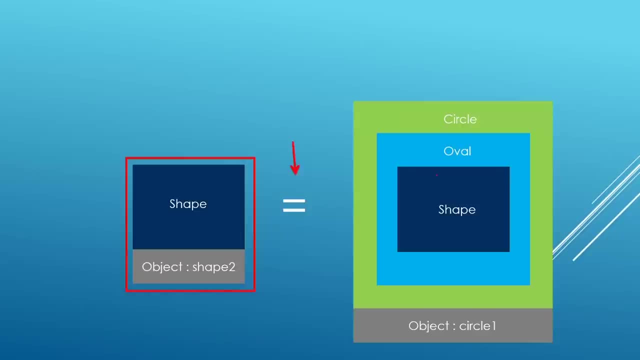 store everything we have to the right of the assignment here and it is going to strip off or slice off everything we don't need and it is only going to leave in the shape part and that's what it is going to assign on our object that we have on the left of the assignment operator here. 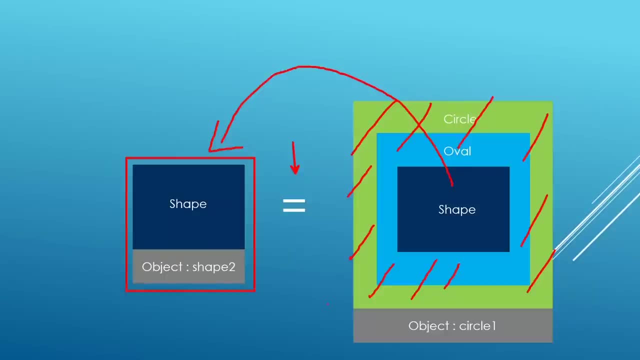 and this is referred to as slicing in a c plus plus terminology. i just want you to be aware of this, and we're going to see a lot of this starting from now. now that you know this, we're going to head over to visual studio, code and play. 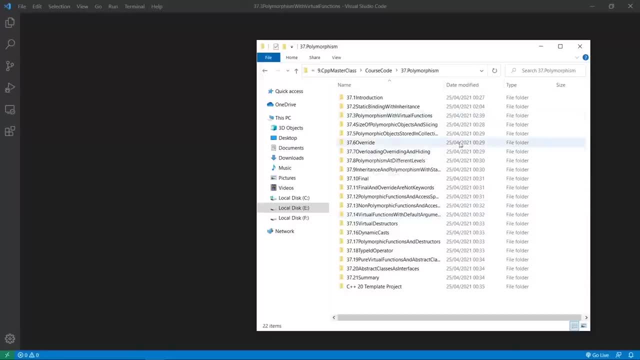 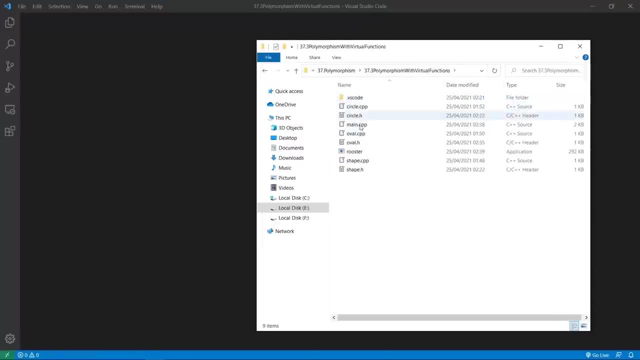 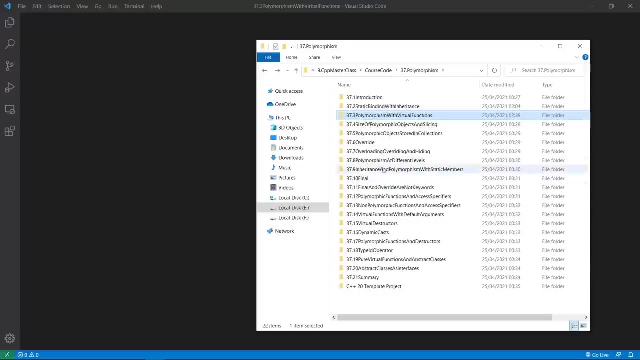 with this a little more. here we are in our working folder. the current project is size of polymorphic objects and slicing. we are going to grab the code from the last lecture, so let's grab everything except for the binary file. we are going to copy everything and we're going to put that in the 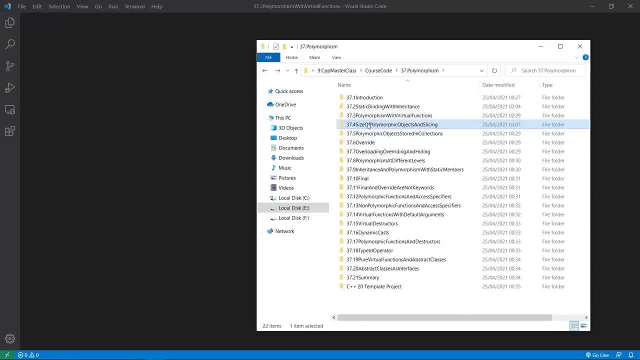 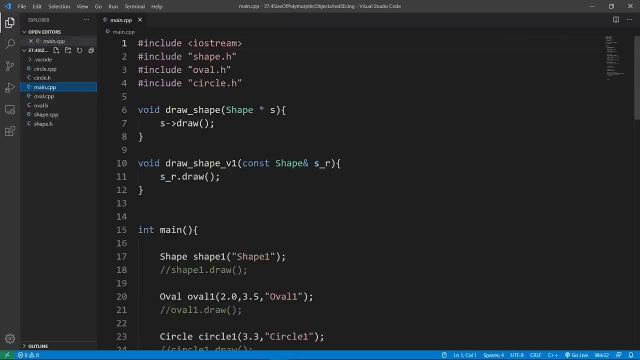 current folder and we're going to open this little guy in visual studio code by dragging and dropping. this is going to give us our project and we can head over in the main cpp file and clean up all the mess we got from the last previous lectures. we can also take out these functions because 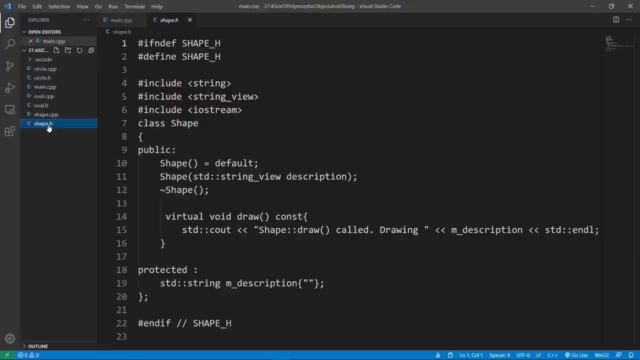 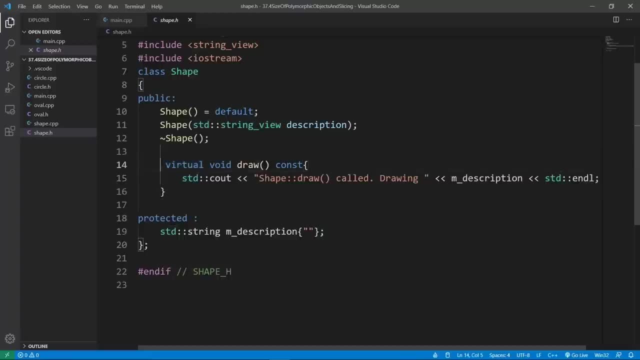 i don't think we need them here and we are going to check out on our classes. notice that we are using dynamic polymorphism because we have virtual functions here. so if we happen to be using base pointers or base references to manage this, we can just copy that and paste it into our project and 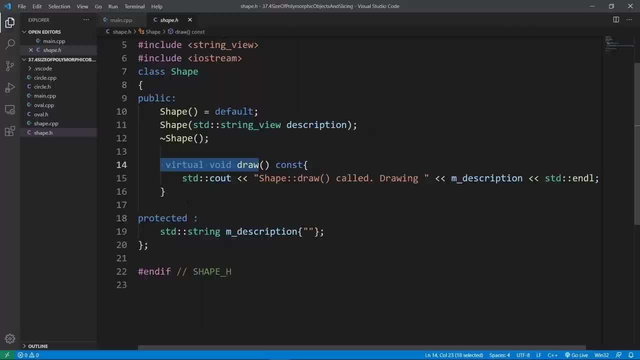 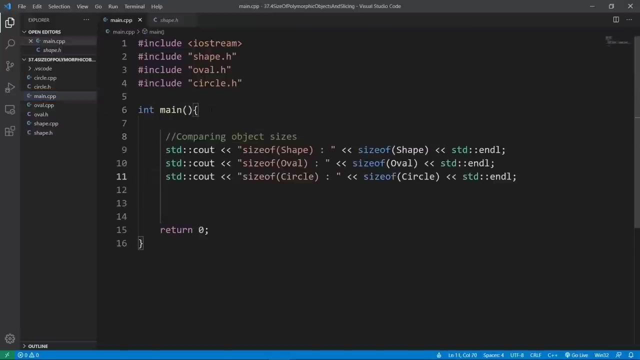 our derived objects, we will get polymorphic results. okay, the first thing we want to see is the size of objects for our classes. here, because we are using virtual functions, let's head over in the main CPP file and we're going to put in a piece of code which is just going to use the size of operator to 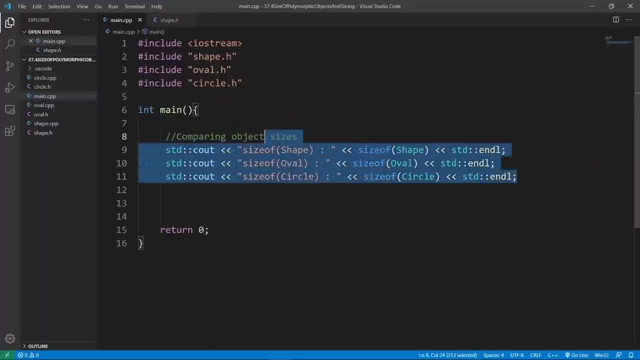 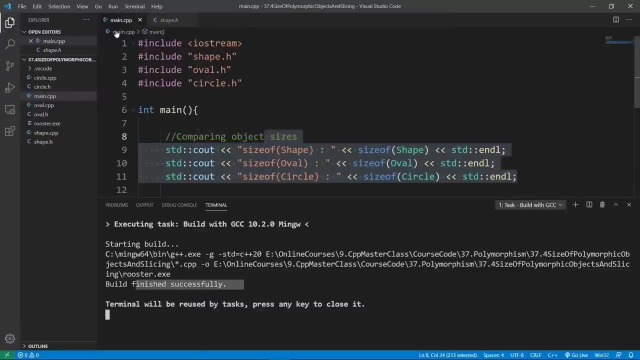 print the sizes of objects of these classes. we can try to build and run this program. we're going to use GCC here. the world is just going to be good. we can bring up a PowerShell window we can use to run these programs. we're going to do. 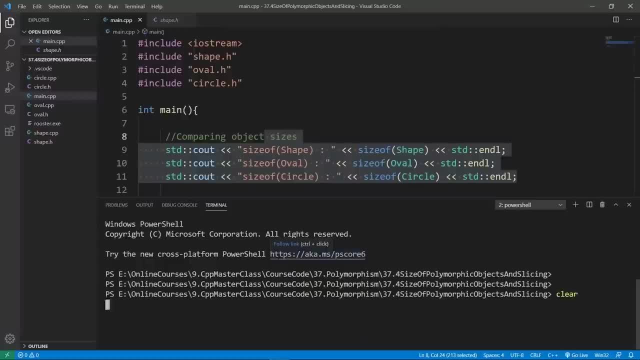 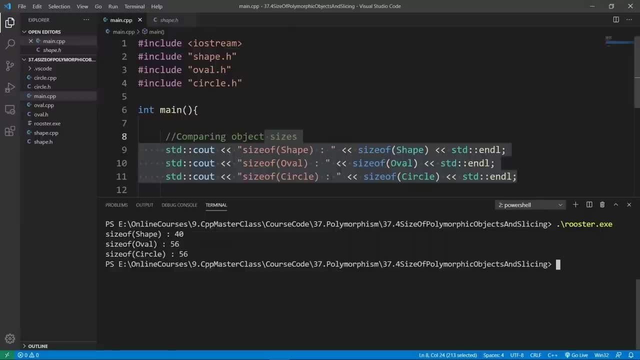 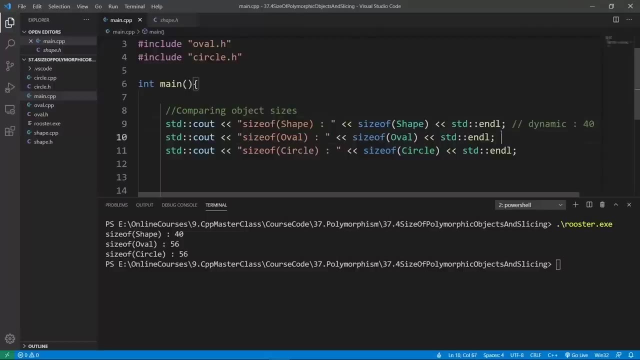 that new terminal. this is going to bring us our window. here we can clear and run rooster. we're going to get 40, 56 and 56. so you see that these are our sizes. so let's say that with dynamic is going to be 40 for the base class. with dynamic, 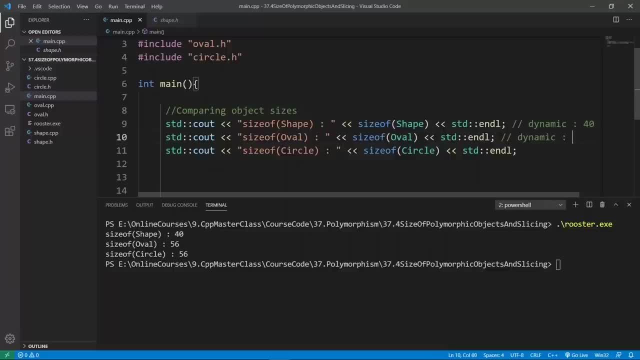 poorly. morphism: we're going to use GCC here. the world is just going to be good. we can bring up a piece of code, which is just going to be good. we can print this and we're going to get 56 for the oval object and we're going to get dynamic 56 for the circle. 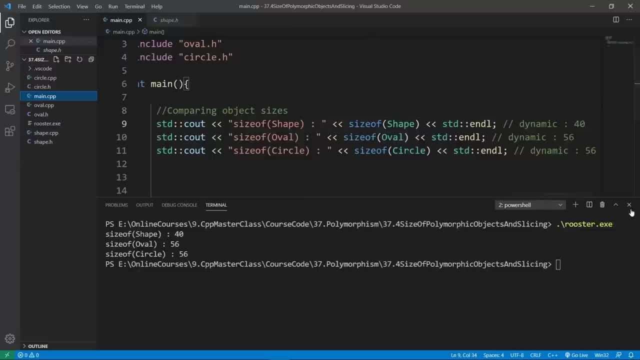 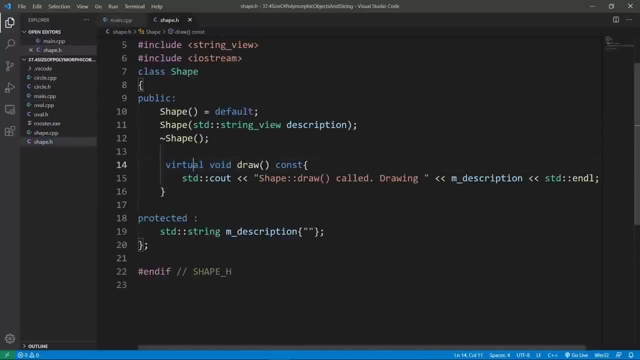 object here. now we're going to remove the setup that uses polymorphism and we're going to see the results that we get. all we need to do is to remove the virtual keyword. here we can comment it out. you can do something like this in shape and we're going to hop over in oval and comment out the virtual keyword. 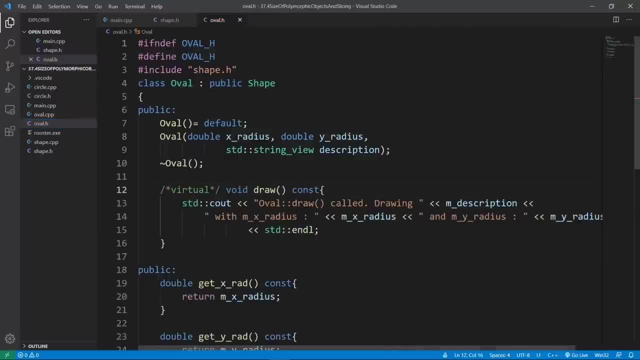 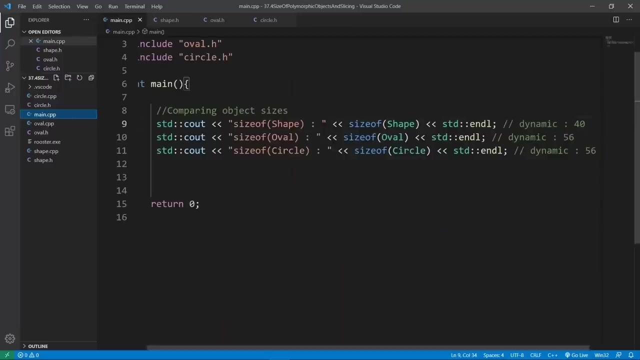 we can do something like this- and this is going to work without removing this completely from our code, because we still need to leave this in as a reference. we're going to hop over to circle and do the same thing, and now that we have this setup, we can hop over to our main CPP file. we're going to see. 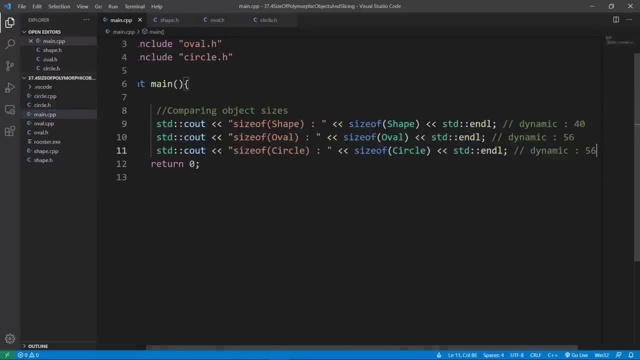 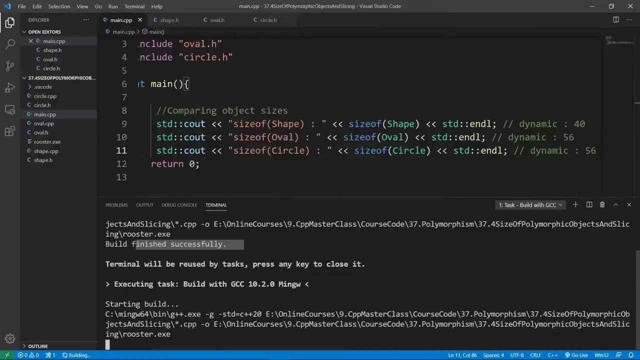 that we don't have any squiggly lines of some kind. so this is going to be accepted by the compiler. but if we build and run this program, we're going to see different sizes. let's see if the program is going to be accepted by the compiler. 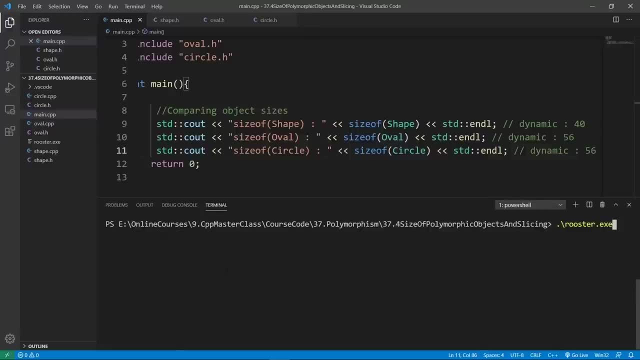 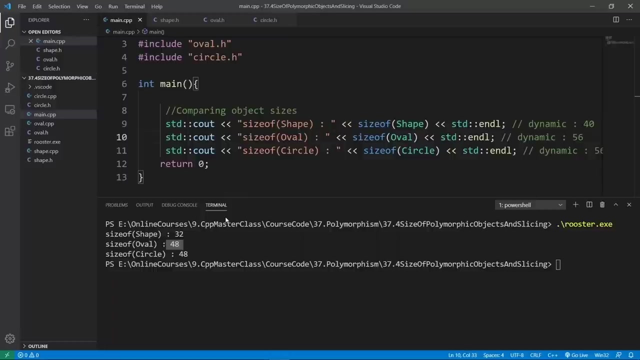 well, this good, it is good. as you see, here we can clear and run rooster. now you see that with static binding, the base object is 32 bytes, the oval object is going to be 48 and hopefully you can see that with dynamic polymorphism, our 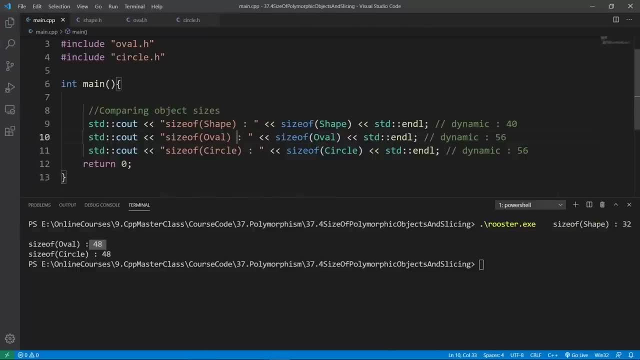 objects are going to be much larger because the compiler has to keep track of the information that allows it to dynamically resolve virtual function calls. that's why our object is going to be larger and the object is going to be. objects are larger with polymorphism and you should know that you are not getting polymorphic. 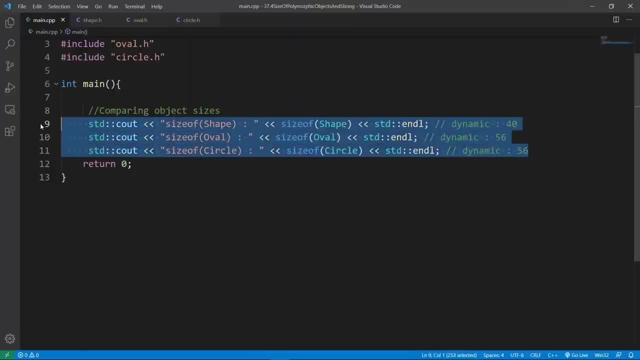 results for free. you are going to be paying in terms of much more memory that you use for your objects in your c++ programs. this is the first thing i want you to see in this lecture. the second thing i want you to be aware of is the concept of slicing, and this is going to happen if you happen. 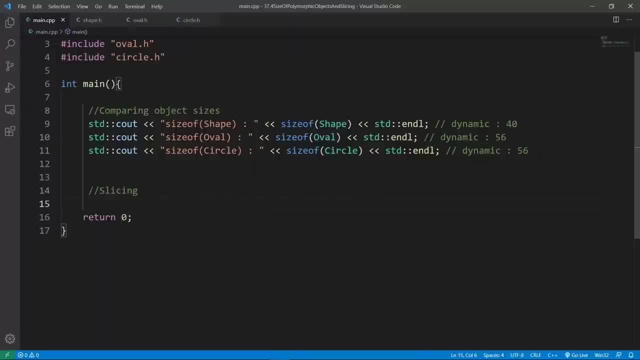 to take a row derived object and assign that to a row based object. let's do something like that: we are going to create a circle object and then we're going to say shape, and say shape here and we're going to say equals circle one. this is something we could do, but notice that the compiler 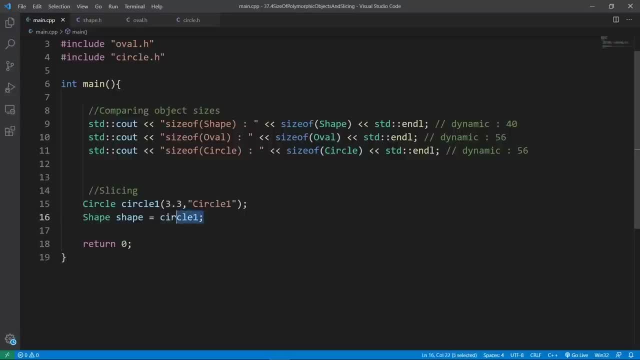 is not giving us any kind of compiler error because we can assign a circle to a shape, because a circle is really a shape. but from what we know in our inheritance hierarchy you can see that the compiler is not giving us any kind of compiler error because we can assign a 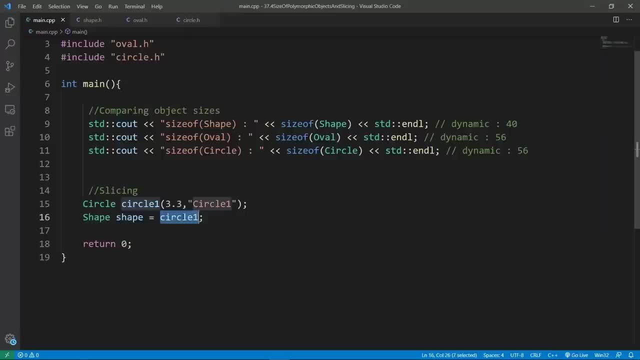 a circle is really much more than a row shape. a circle has oval information in it and it also has circle information in it, so it is really much larger and much wider than a shape object. but the compiler is going to see that we are trying to assign a circle to a shape and it is going to be. 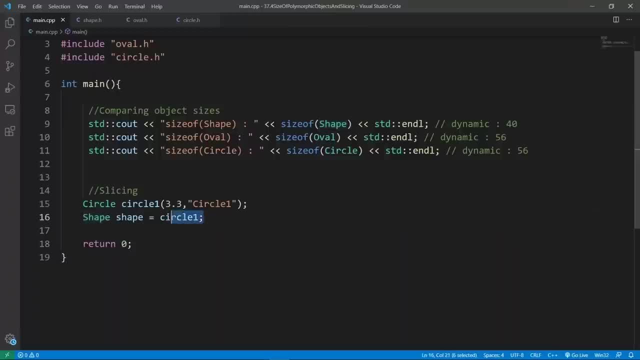 smart enough to know that we don't really need oval and circle information in our shape object that we are storing here. so the compiler is going to slice off circle and oval information and it is going to leave in shape information and that's the only thing we will be able to use. 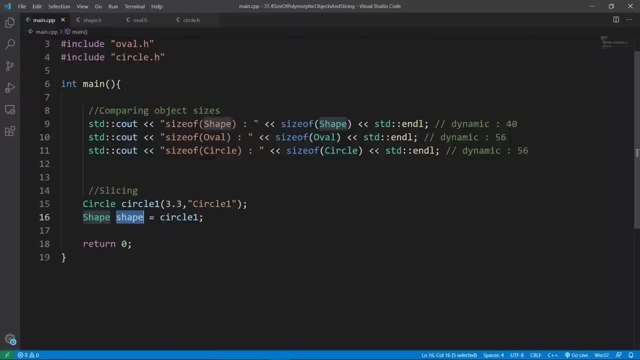 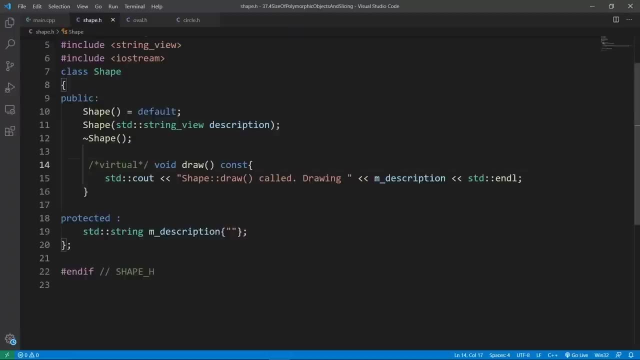 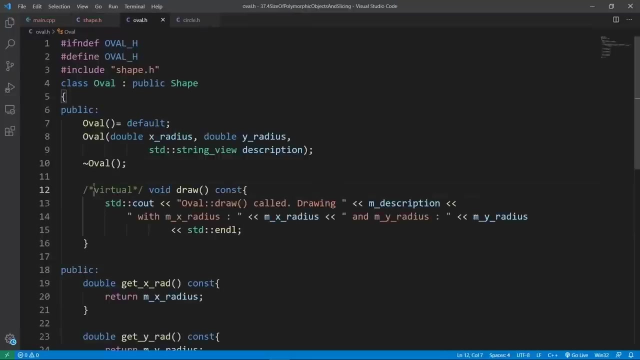 with this shape variable that we have in our c++ program. so if we say shape draw, you can try to guess what we are going to get. and let's go back and re-enable polymorphism, because some of you might think we are going to get polymorphic results with this setup here. that's. 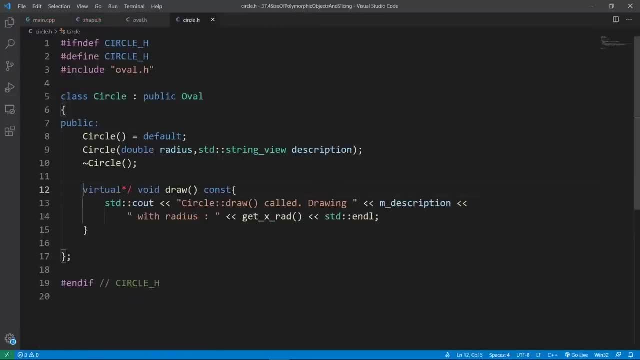 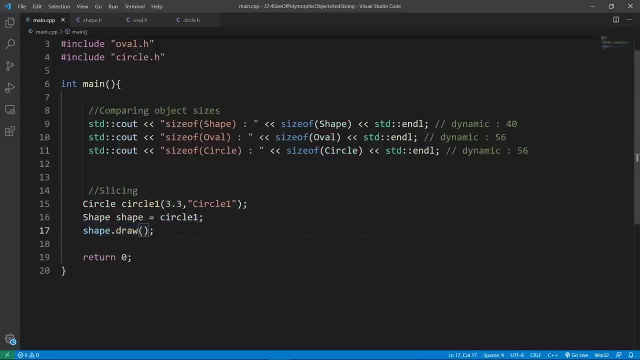 not what we're going to get because we are not going through base references or base pointers to do what we are doing in this example on slicing here. so because we are not using base references or base pointers in this line here, the compiler is going to see that these are row objects and 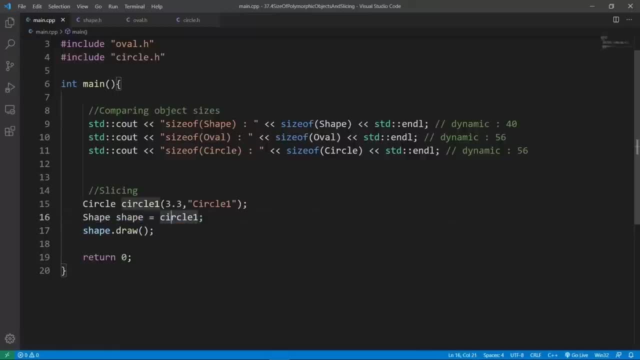 it is going to do slicing and slice off things we don't need in our shape variable that we are setting up on line 16 here. so if we call the draw method, this is going to call shape joe. it is not going to do dynamic polymorphism here. you should be aware. 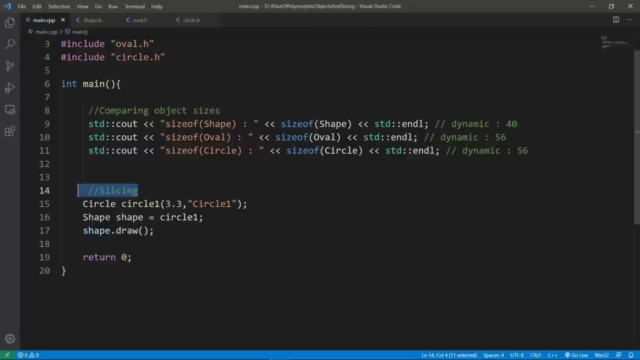 of this. if you're not using the base pointers or references and you hope to get dynamic polymorphism results, i hate to break it to you, but you're going to be disappointed because the compiler is going to slice off derived class information and all you're going to be left with is base class. 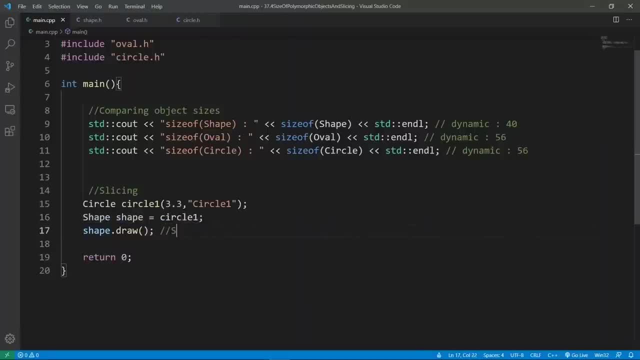 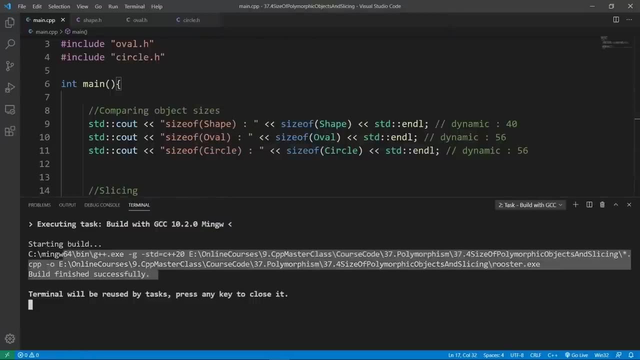 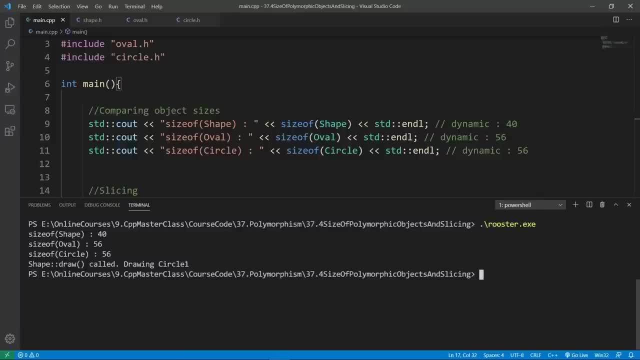 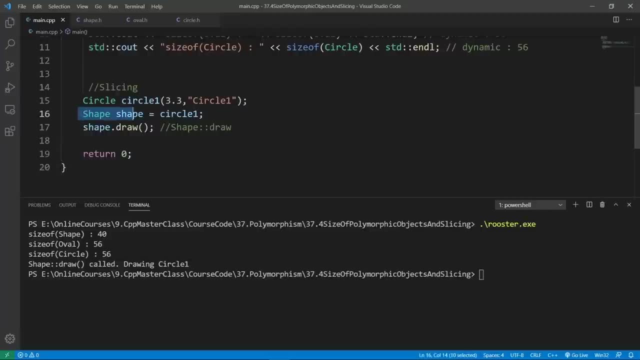 we cannot clear and run rooster, you're going to see that it is going to say shape, draw. even if we tried to assign a circle to a shape here. this is going to disappoint us because this is really going to slice off circle and oval information and it is just going to leave in the shape nucleus. 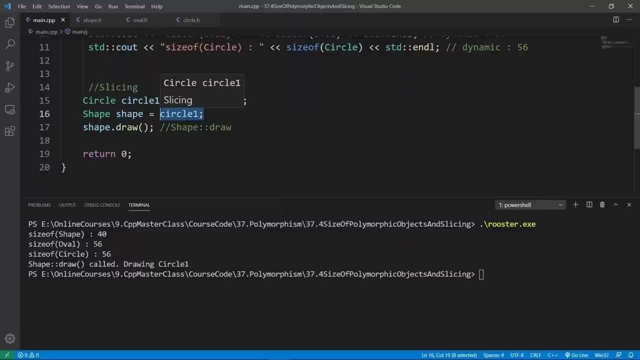 that we have in our circle object here, if i can say it like that. this is really all i had to share in this lecture. i hope you found it interesting. we are going to stop here in this lecture. in the next one we're going to see what happens if we try to store polymorphic objects in collections. 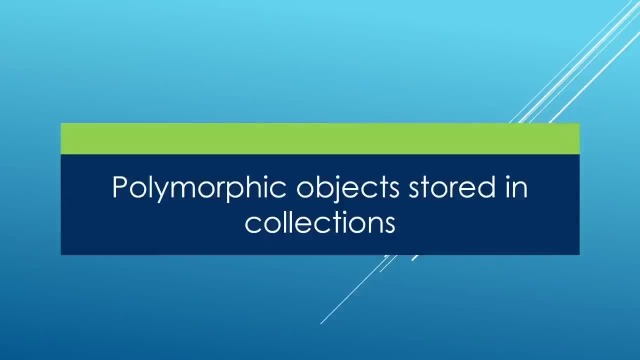 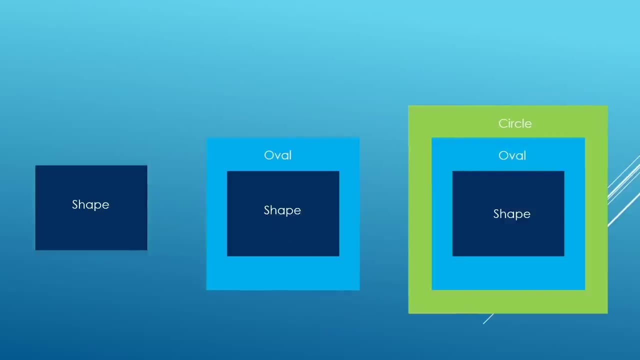 go ahead and finish up here and meet me there. in this lecture we're going to explore what happens if you try to directly store polymorphic objects in a collection like an array. in the last lecture we have seen that if you assign a derived object to a base object, the data from the derived object is going to be basically sliced off. if you assign 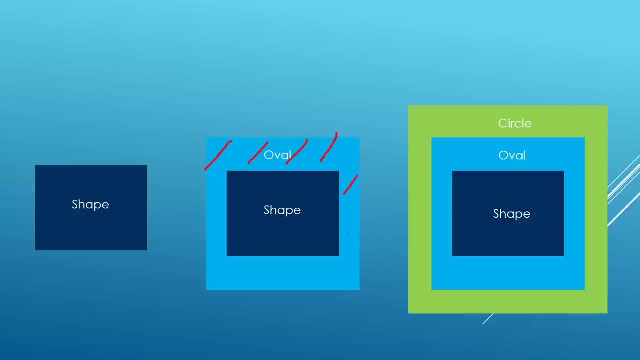 an oval to a shape, the oval part of the object is going to be sliced off and we're going to be left with only shape data that we assigned to our shape object. we saw that this was referred to as slicing in c plus plus, and the same is going to happen if you assign a circle object to a shape. 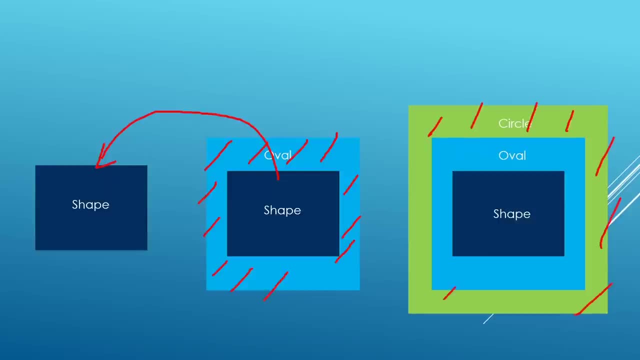 the circle information is going to be sliced off, then the awful information is also going to be sliced off and we're going to be left with the inner shape part that we assign to our shape object here. now i want you to see that this can happen indirectly in ways that you might not. 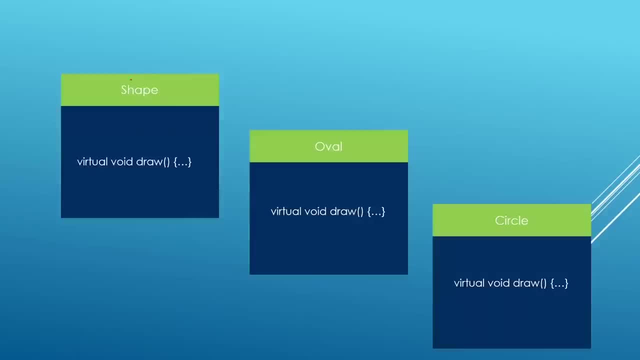 expect, and we are going to use our inheritance hierarchy again. the base class is going to be shape. we're going to inherit from that and get oval, and we're going to inherit from oval and get our circle class here. so let's look at a piece of 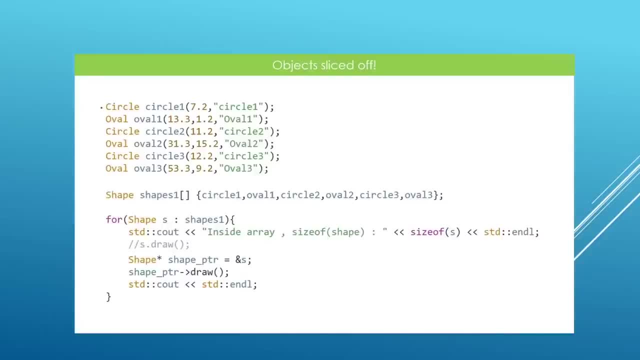 code. here we are creating a bunch of objects. we have a bunch of circles and ovals and we are setting up an array that is going to directly store ship objects. but what we are doing is storing our pre-created objects in our array. here, and from what you already know, if you store objects in an array, 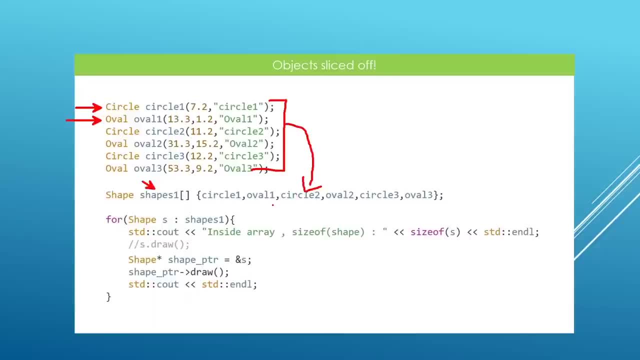 like this. this is going to create copies, even if you can't see that directly. so what we have in our array here is not so. what we have in our array here is not any kind of direct reference to the object we have on top here. these are just copies. and notice what is happening. we are copying derived. 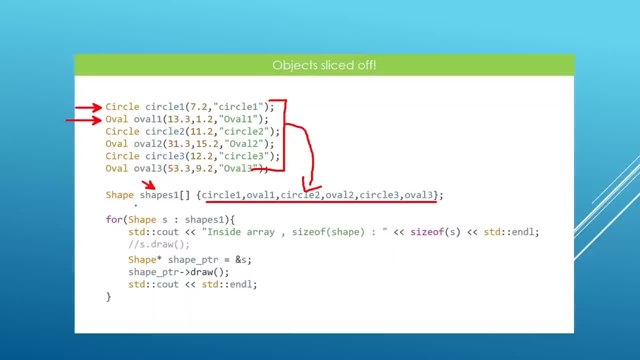 objects in spots that are designed to store direct shape objects. and you might guess what this is going to do. this is going to slice off circle and oval information and only shape information is going to be stored in this array here. so if we happen to loop through this array, 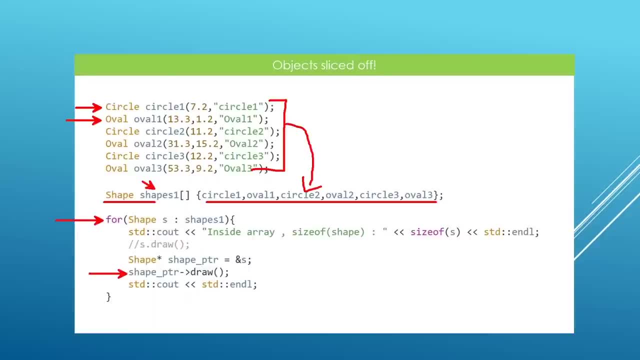 like we do here and try to call the draw method. this is not going to call the most specific draw method for circle or oval. this is just going to call the shape version of our draw method here. this is something i want you to see. okay, some of. 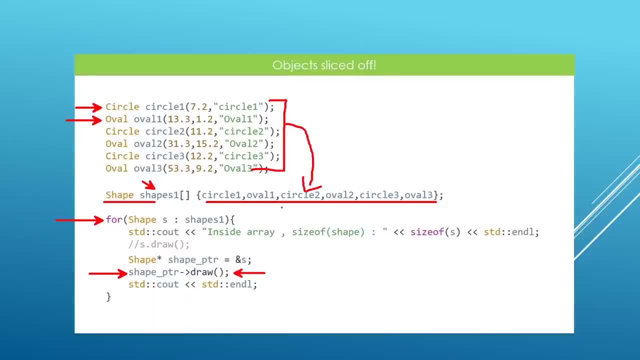 you might say: what if i take my shape information in here and assign that to a pointer and then go through that pointer to call the draw method? well, i hate to break it to you, but the moment your data is sliced off in a situation like this, you'll never get that data back. so even if you try and 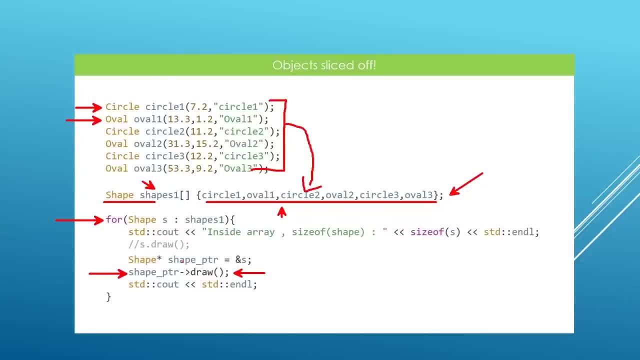 take the object and assign that to a pointer or a reference, you're never going to get polymorphic data again. the data has been lost permanently and you never get that. so even if you try to go through a pointer or a reference to manage your object that we have in this array, if we call the draw method, we won't get polymorphic behavior. we will. 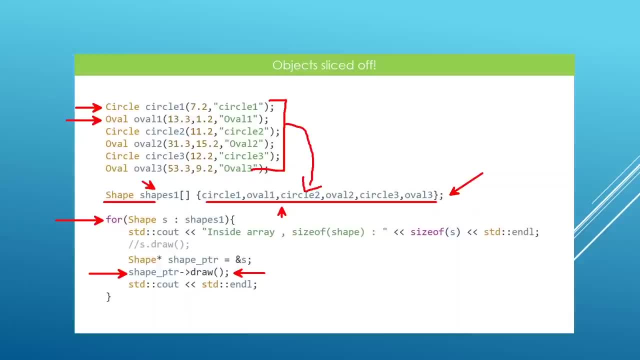 get to the shape version of our draw method called. so the data has been sliced off permanently. if we store our derived objects in an array like this, or even if we directly assign a derived object to a base object, this is going to slice off the data and we will. 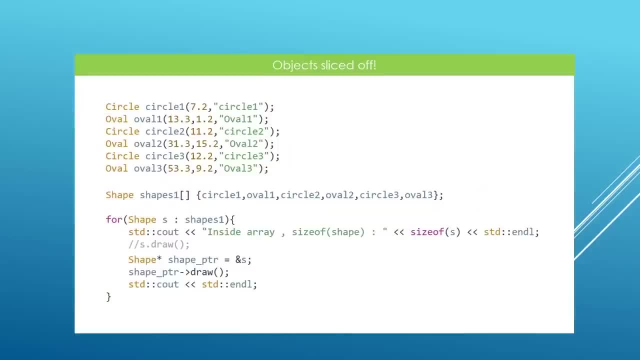 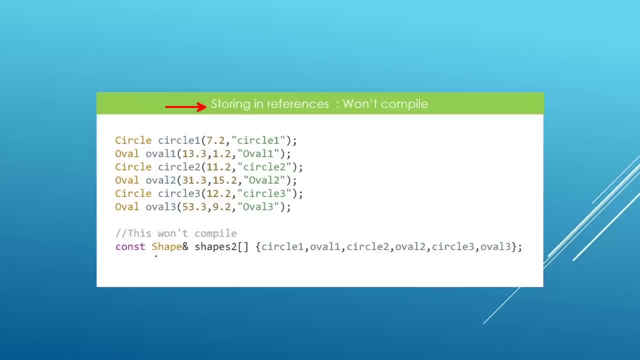 never get it back. anyway, you should really know this. okay, anytime i try to explain this, students mostly come up with this question: what if i try to store references in my array and do something like this? now, this is not going to work and this is not even go past the compilation stage of your 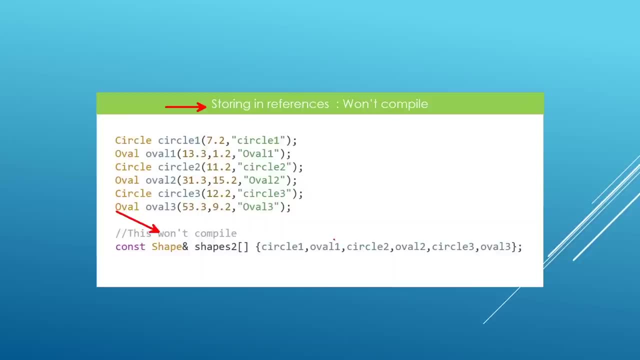 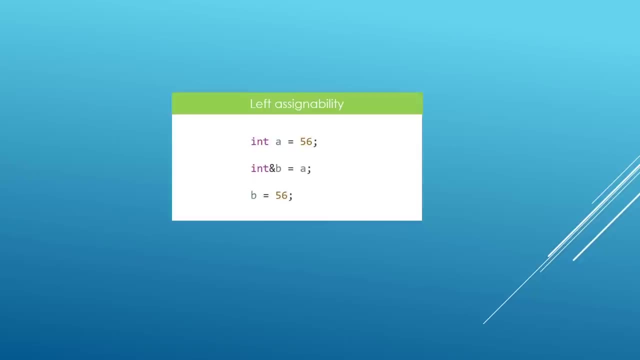 lab. the reason is we can't store references in a collection and the reason has to do with the left assignability rule. you can't assign to a reference and change the reference to store somewhere else. and to really drive this home, let's look at this example. here we have a variable called a. it is of 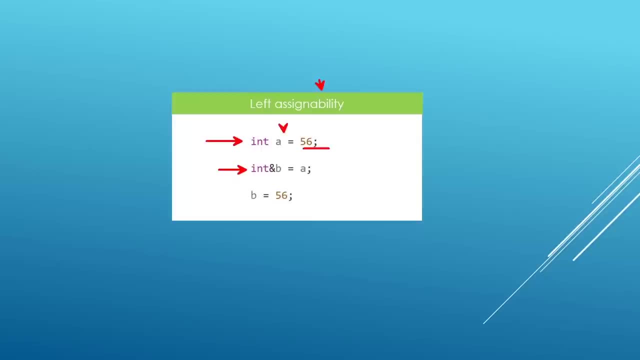 intertype and we have a 56 value inside and we set up a reference which is going to be referencing the data we have in a and down on this line. here we try to change the data in our reference, but this is not going to be changing where this reference is pointing to or where this reference is referencing. this will. 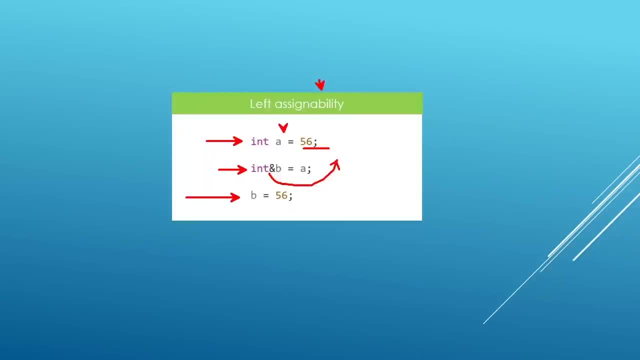 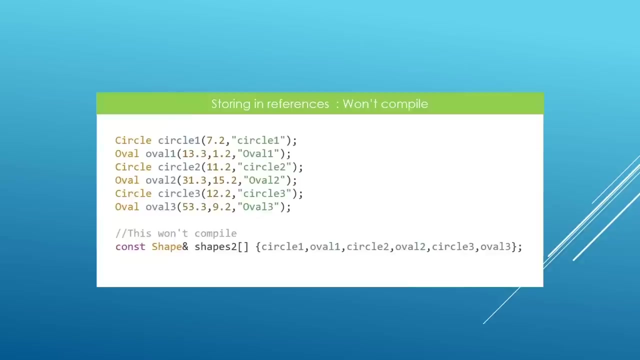 merely be changing the values in our reference here, and once we have this reference, we'll never be able to change where it is pointing again. so from this, hopefully you can understand that references are not left assignable. you can't store things that are not left assignable in an array, because an array is designed to modify. 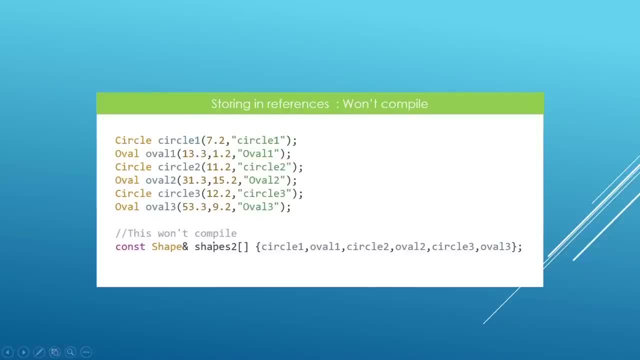 the data of what is stored inside. so if we set up an array like this, the compiler thinks that at some later point you will want to assign other data to what is already stored in this array and there is a hard requirement on the data you store in your collections for the type of that data. at last to 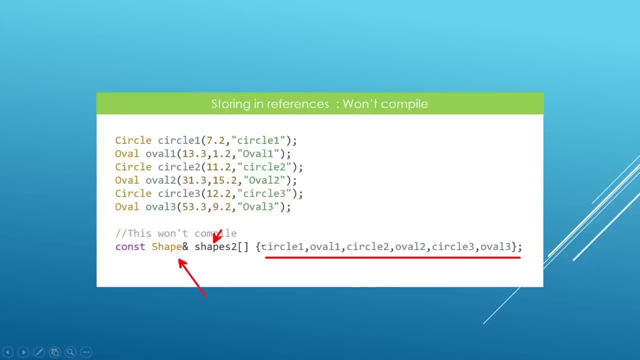 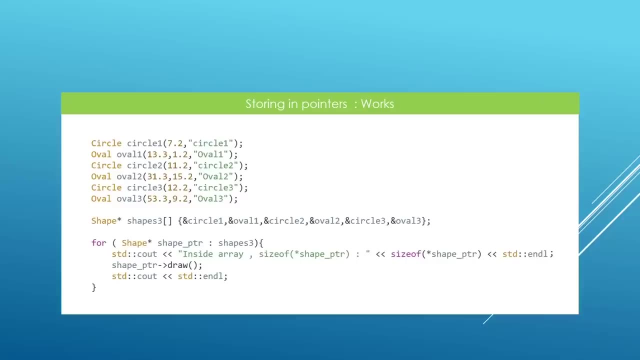 be assignable and references are not left assignable, so we can't store them in a collection like this. if we're trying to do this, we're going to get a compiler error. but again, some of you are going to say: what if we store in pointers? well, this is going to work. this is the basic working. 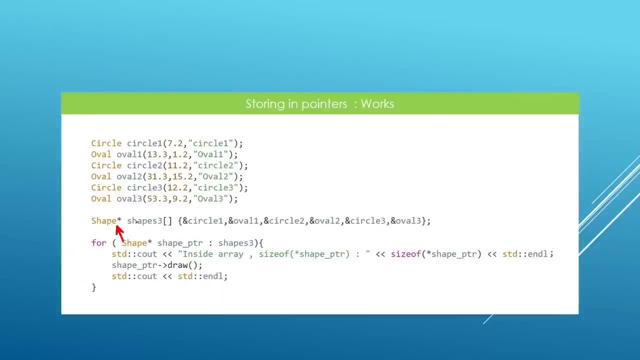 principle of polymorphism, going through base pointers to manage derived objects. this is going to use polymorphism and here we will get to the most basic draw method called. so if our object is a circle, we will call the draw method on the circle object. if it is a novel, we're going 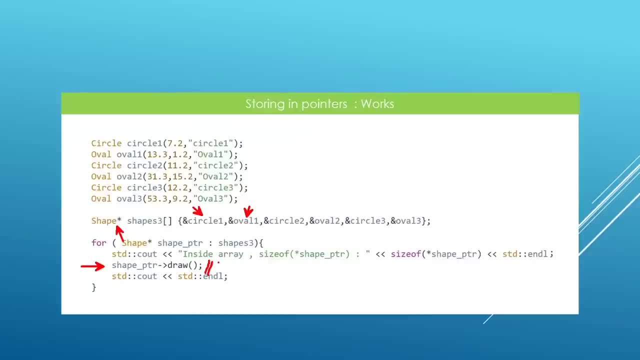 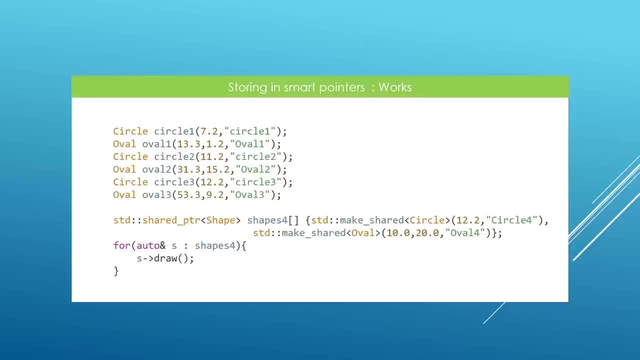 to call the draw method for the over part of our object. here this is even going to work if we go through smart pointers. so if we do something like this and storing smart pointers and create our smart pointers on the fly in our initializer, here this is going to work, because really a smart 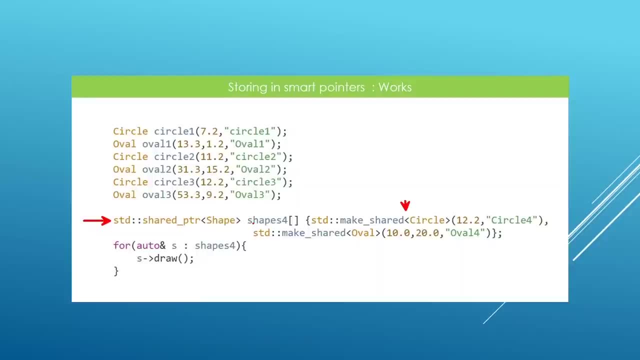 pointer is a wrapper on top of a regular row pointer in c plus plus. so again, the message here is that you need to be careful on what you store in your collections. if it is a raw piece of data, your data is going to be sliced off. if you store derived, 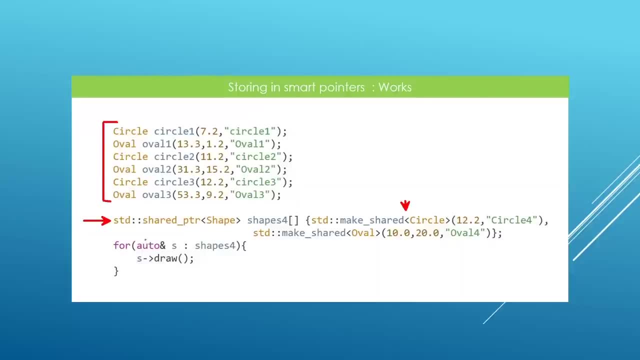 objects in a collection that is designed to store base class data. if you store in references, that's not even going to compile. but if you're storing any kind of pointer row or smart, this is going to work, because polymorphism is designed in the first place to work with base pointers that are managing derived objects and 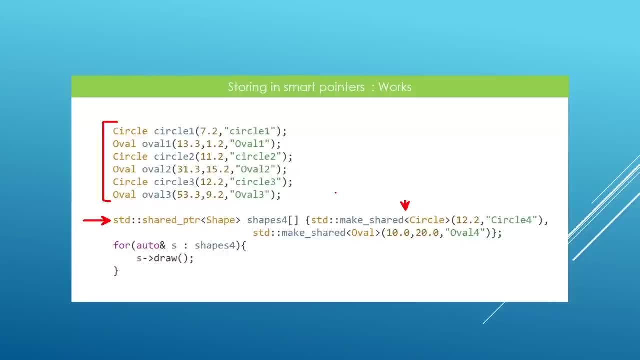 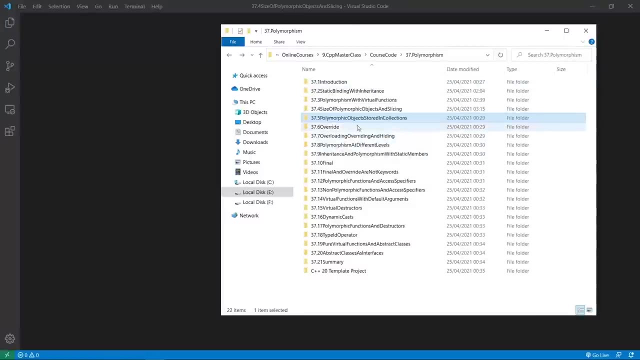 this is really cool and I want you to be aware of this. now that you know this, we're going to head over to Visual Studio code and play with this a little more. here we are in our working folder. the current project is polymorphic objects stored in collections. we are going to reuse the code from 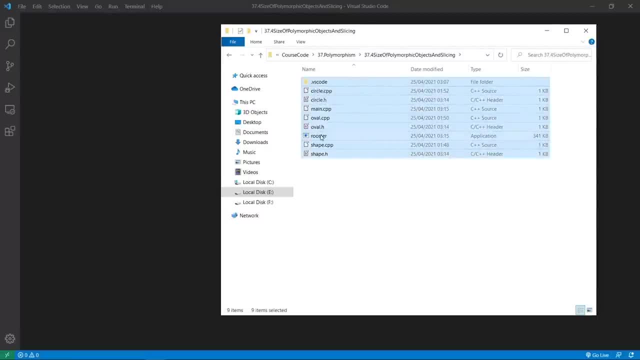 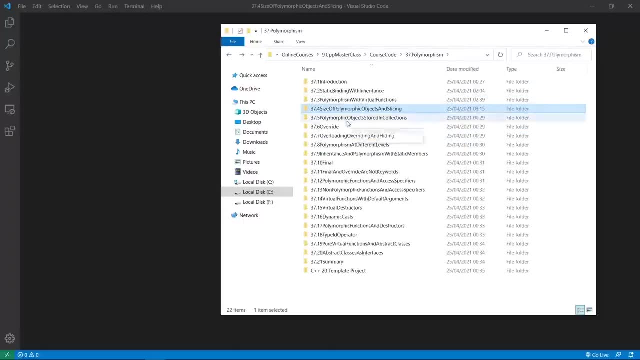 the last lecture, because we need our inheritance hierarchy here and this is going to serve us just well. well, we're going to copy this and we are going to head over in our current project and put in our code and then we're going to open this in Visual Studio code. pretty quick, let's do this. 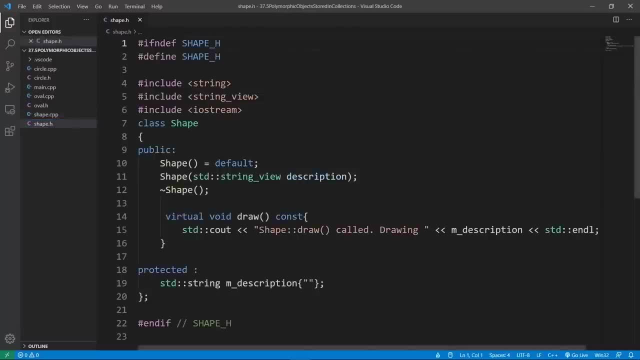 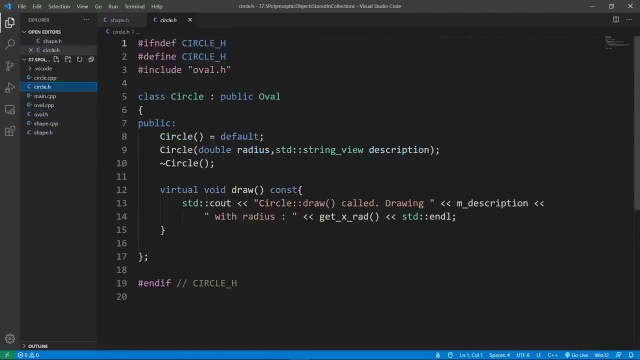 this is going to give us our code, and we have our shape class, which is really what we already know. we have our oval class and we have our circle class. take a good look at this, and what we want to see is what happens if we use different kinds of setups to store objects. 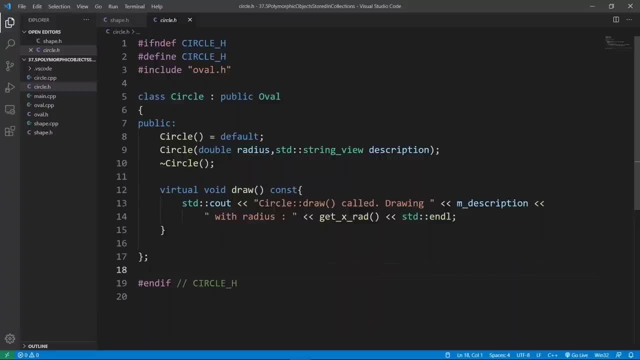 of this inheritance hierarchy in a collection like an array. let's go back to our main cpp file and we are going to take out what we have it. here we're going to set up what we're going to be using in this lecture. we are going to set up a bunch of objects that we're going to be using here. basically, 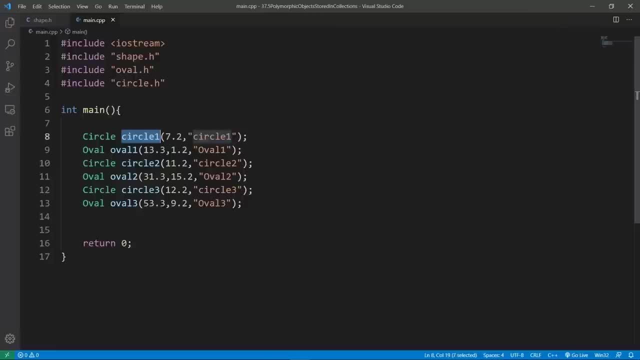 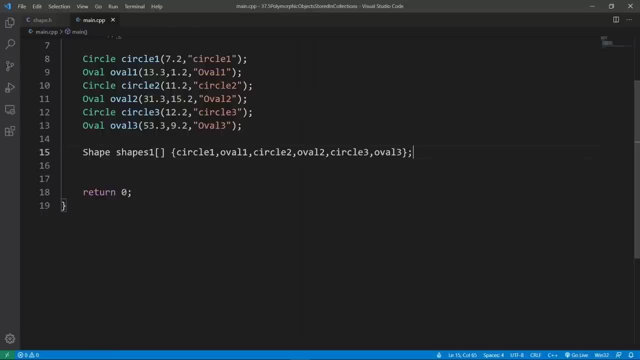 a bunch of circles and ovals. we can close the left sidebar here and have some more breathing room. after this we're going to set up an array which is going to store copies of this object in this array here, which is called shapes one, and after this we're going to try and loop through. 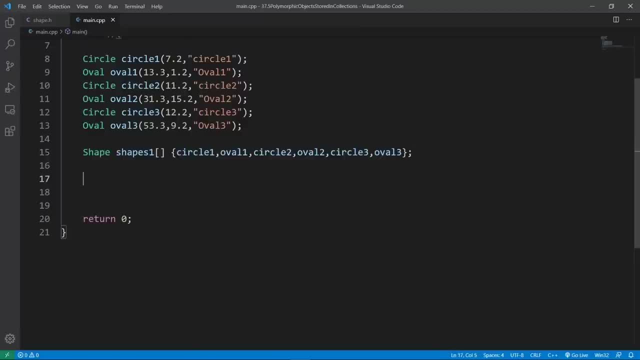 this array and try to do things with it. for example, we can say for shape and we may want to call the draw method on our copy here. so for example, we can say s and say draw, going to see what happens here. and let's say references, because we don't want copies in our range based for a loop. 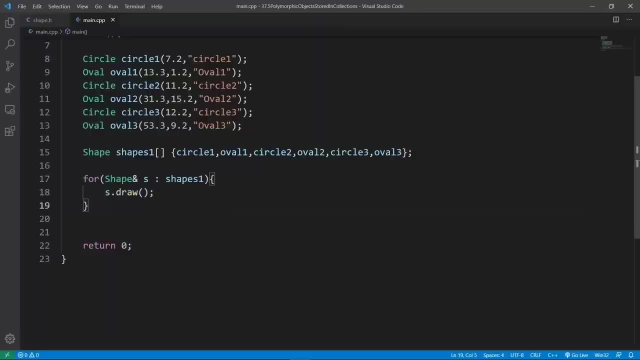 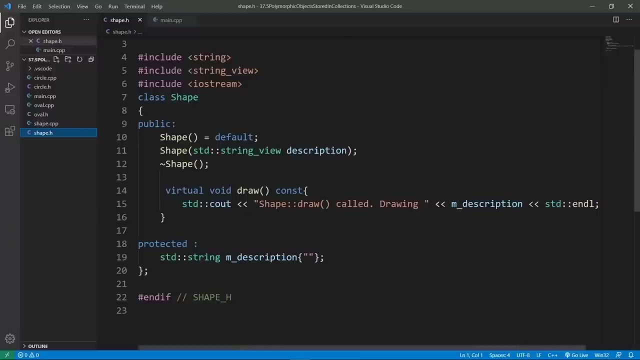 here. so this is going to avoid copies we do in this loop and we're going to be directly referencing whatever we have in this array here. now, what do you expect to get? we have derived objects in this array and with the setup we have here, because we are using virtual functions, one would expect to get polymorphic behavior. so here: 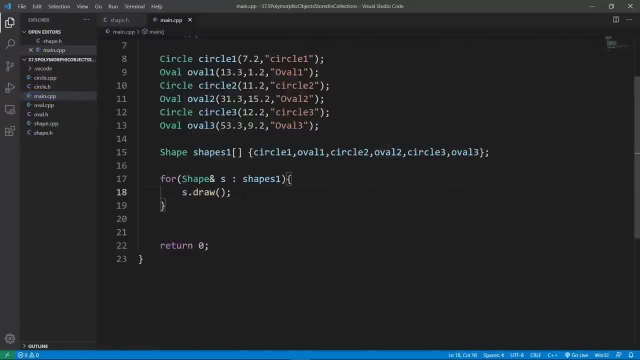 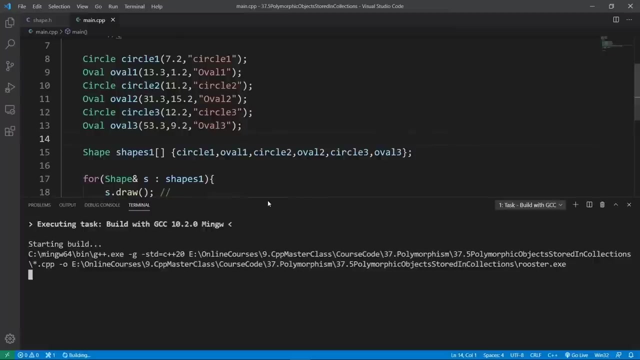 we would expect to get the Joe versions in circle and awful to be called, but that's not what is going. shape versions of our Joe methods. let's try and build and show you this. we're going to build with gcc, our favorite compiler. the build is going to go through. we can kill this and bring up a. 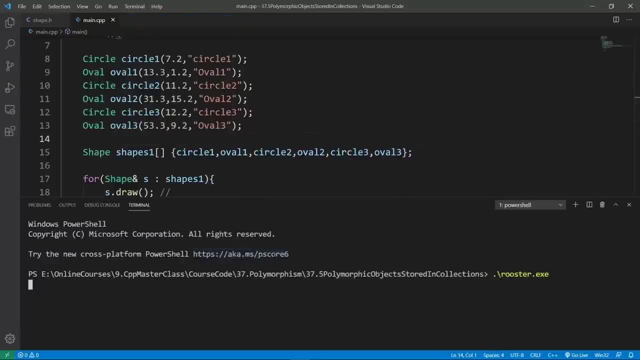 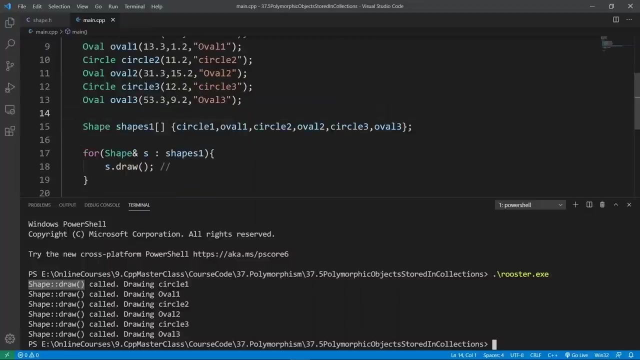 PowerShell window to allow us to run our program. we're going to say rooster here and you're going to see that we are drawing circle one over one, circle two over two, circle three over three. but we are calling the shape versions of our Joe method, and the reason is: 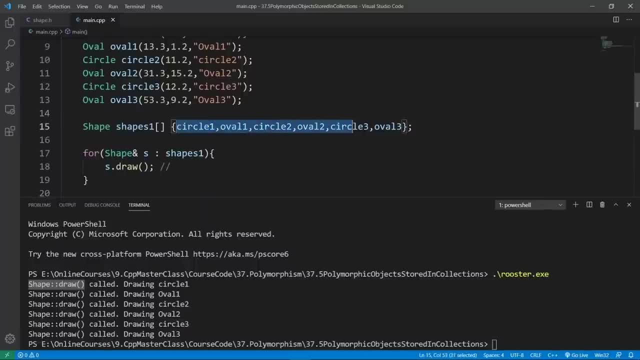 we are slicing off derived class information in our objects the moment we try to make a copy and copy in a spot that is designed to store objects of the base class. so this is basically what we saw in the last lecture on slicing, but it is disguised because we are storing data in an array. 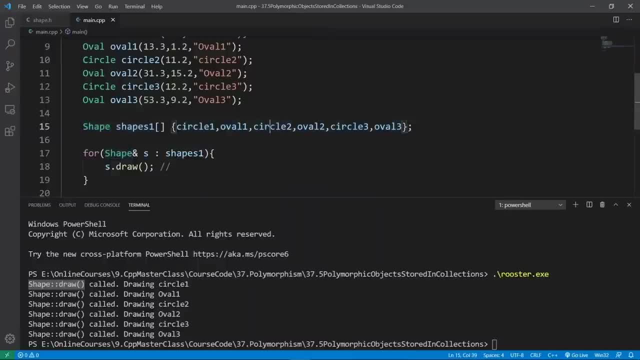 and when you store data in an array like this, you're going to be making copies and storing copies in your array, and in any copy you make you're going to be basically slicing off oval and circle information and only storing in shape information for our objects here. this is what the compiler is going. 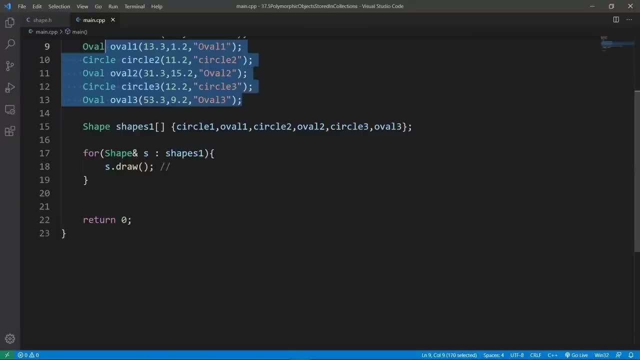 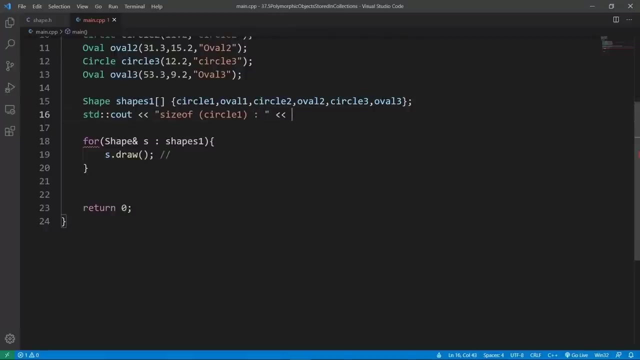 to do and to really try and prove this. we can try and print the size of these objects and see the sizes of these objects in this array here when we loop. so for example, we can say: stdc out size of circle one. do we have circle one? yes, we do. so we're going to say size of circle one here and we're going to put it size. 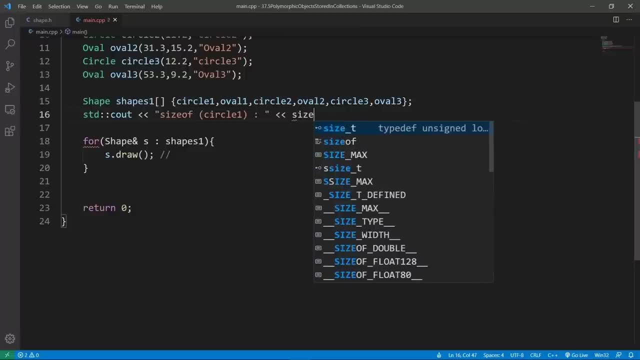 information out here to be seen by everybody. we're going to say size of circle one, and we're going to print it out. and we are also going to print the size of whatever iteration we are at in our loop here. that's the first thing we're going to print. and we're going to say size of object, and we're 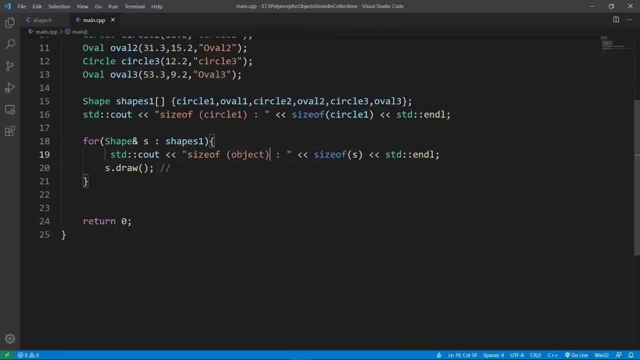 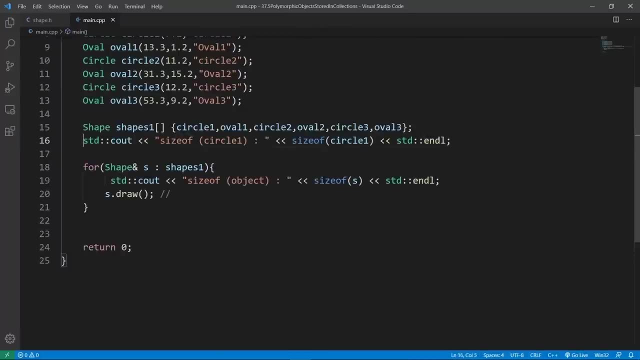 going to say size of s. this is going to do and we're going to loop and see: the information we have on the outside is the same as we have on the outside. again, we are printing this information on the direct object, which is really not yet in our array and in fact we can. 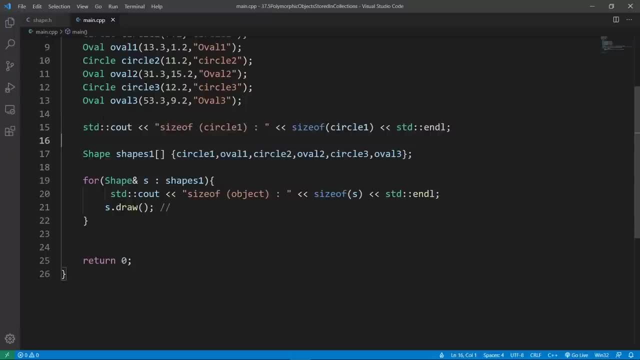 bring this in front of our array to make this super clear, and in our loop we are printing information on a copy that we have in our array, because this is the real deal we have in our array, because this is a reference. hopefully this is going to make sense and prove to you that we are going to be working with derived objects. 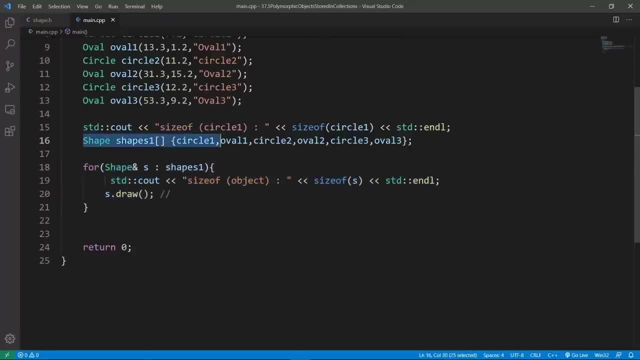 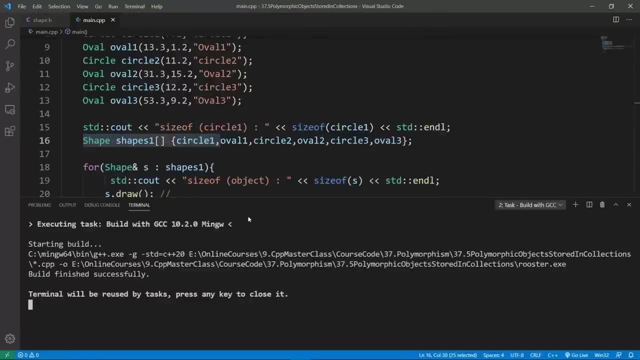 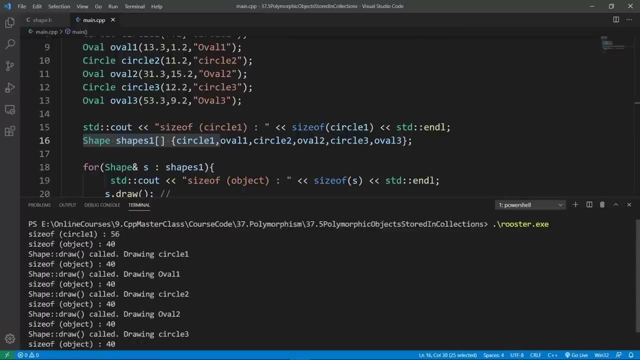 and that the data is going to be sliced off if we copy the data in our array here. this is what I want you to see. so we're going to run this again, we're going to pass this through gcc. the world is going to be good. we kind of clear and run rooster. now let's look at what we have here. size of circle. 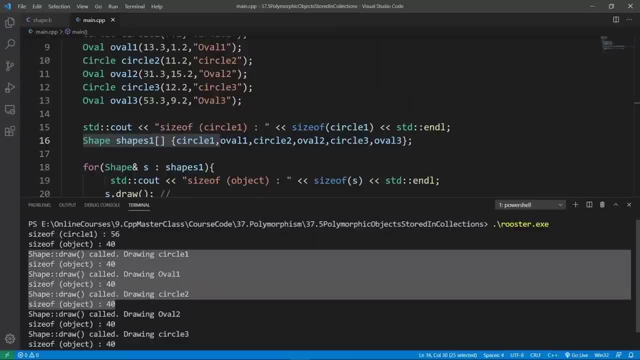 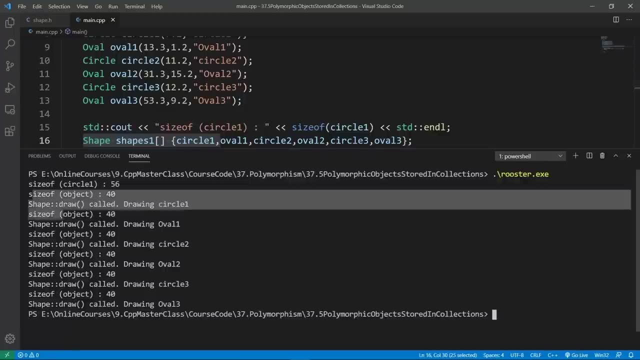 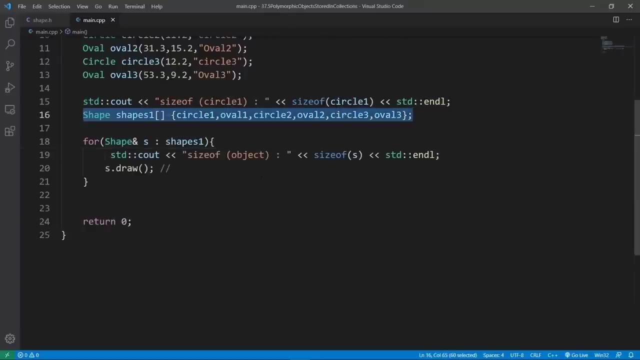 one is 56, but you're going to see that the size for all our objects in our array has shranked to 40 because derived class information has been sliced off the moment we copied our data in our array here and this is what I want you to see and I think we can even see. 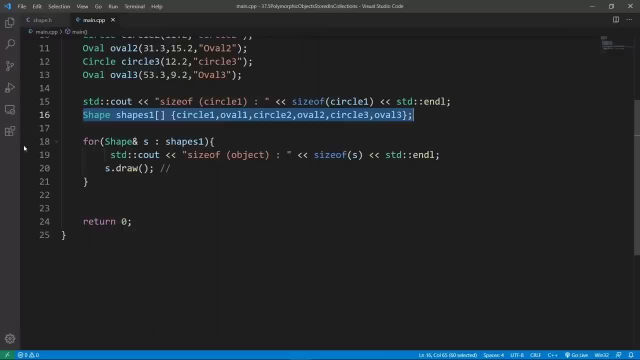 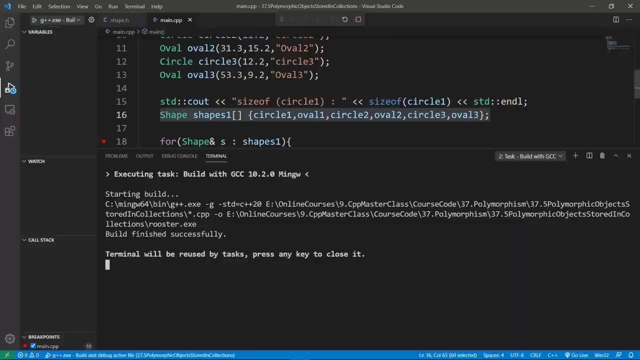 this: if we go through our debugger, for example, we can put a breakpoint here and open our run top, and if we try to run our program through the debugger, the build is going to be good and the binary is passed into our debugger and we're going to hit our breakpoint in a minute. so let's wait for this. 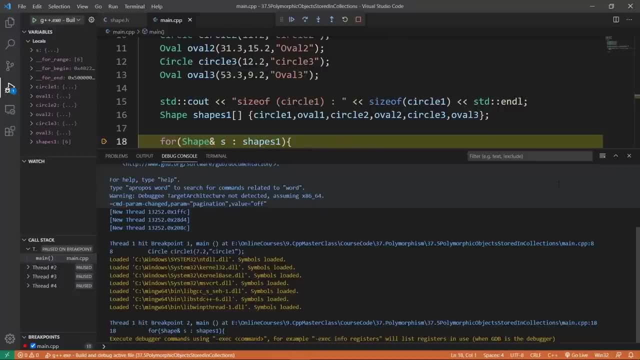 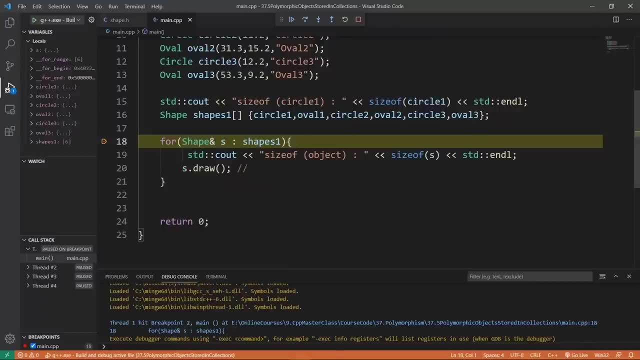 and we have hit our breakpoint here. but what we can do now is look at our local variables on the left. let's look at our array. the array is called ships and if we go up we're going to see our ships- one array- and we're going to see that we have five indexes here because we have six elements inside. we 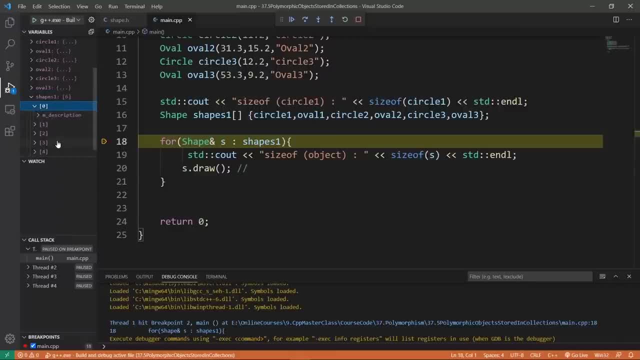 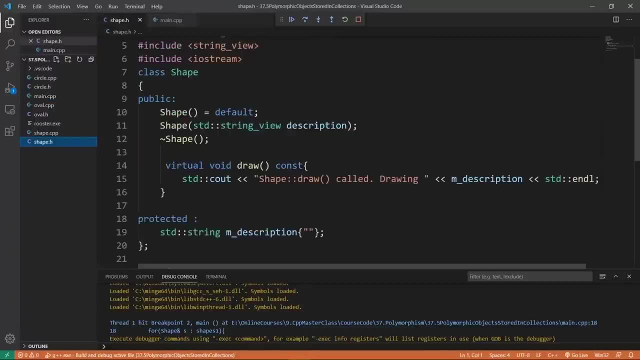 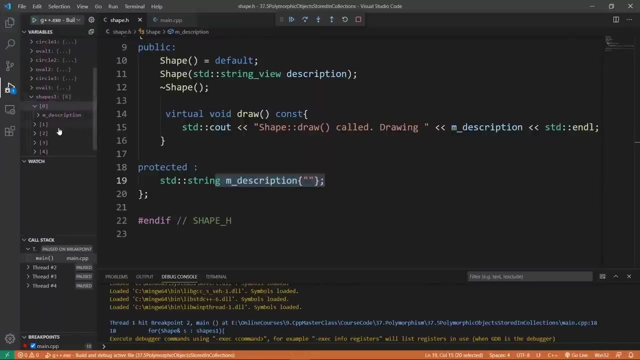 can expand and see what we have at index zero and you're going to see that we just have description data because this is a shape. if we go back in our class, we're going to see that the only thing we have in our shape class is really a description member variable and it is what we see in our array. 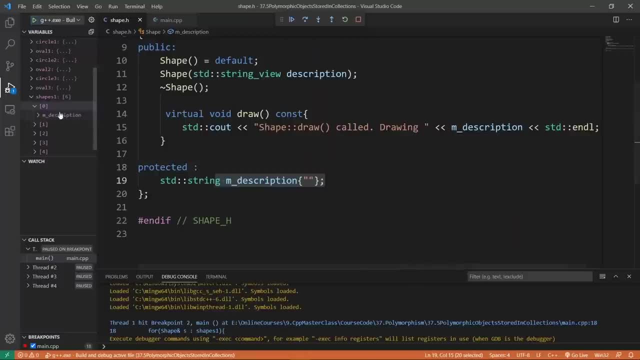 here just description information, because this is a shape object and we have lost or derived class information and this is really cool. but if we go on top and, for example, expand circle one, we're going to see that we have a novel part of us and we have a shape part of us. but these things 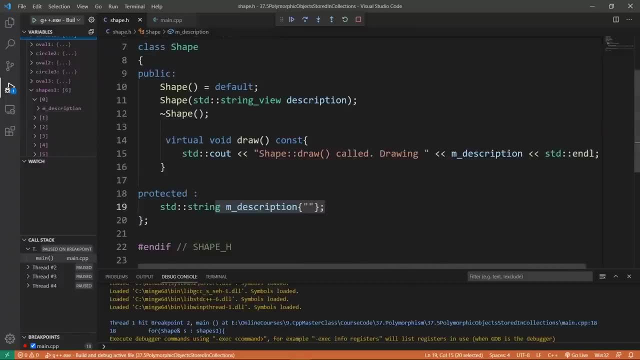 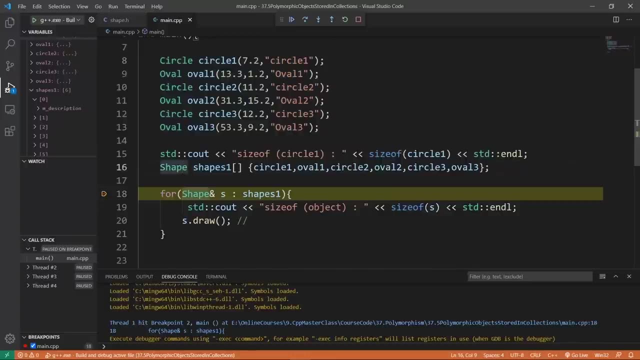 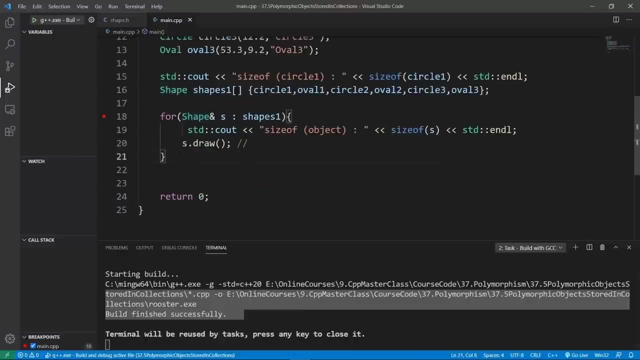 have been stripped off in our array. when we slice off the data from derived objects to only store shape information in our array here. I hope this makes sense. now we're going to kill our debugging session because we don't need this anymore and we are going to comment this out and see some other. 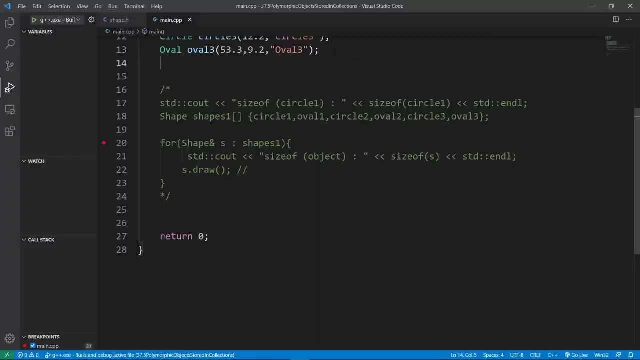 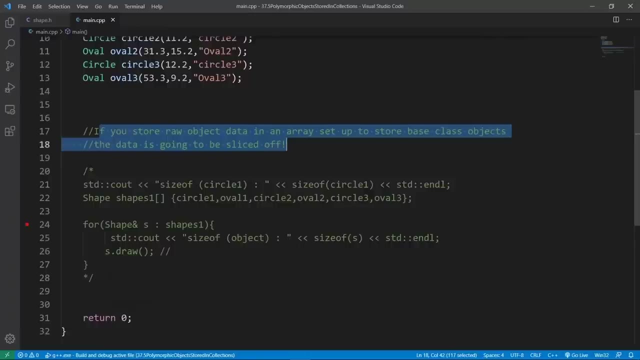 things. so we are going to comment with our data here. we're going to say: if you store row derived objects in an array which was set up to store base class object, the data is going to be sliced off. this is something I want you to know, but some of you 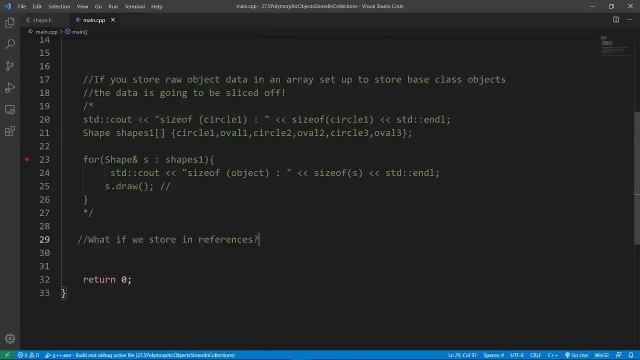 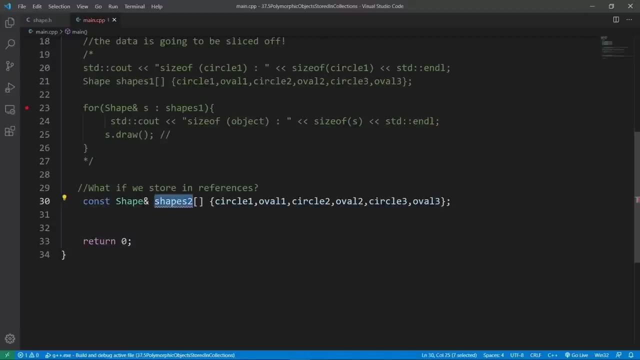 are going to say: what if we store in references? okay, so let's try and do that. we're going to set up a piece of code like this and we're going to set up an array called shapes too, and this array is going to be basically storing references to the objects we have on top here, and we're going 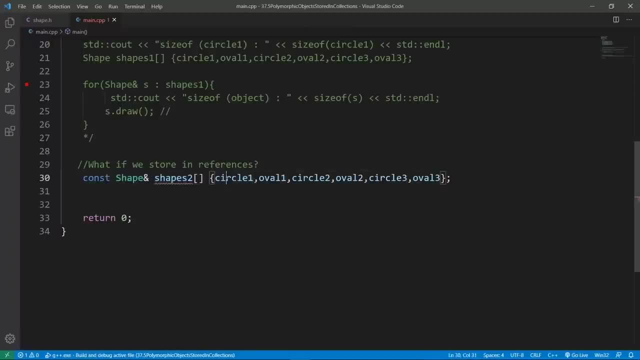 to see what happens. you notice that we have a squiggly line already and this is saying: this is not going to work because references can't really be stored in collections. again, as we saw in the slides, the reason is because references are not left assignable and they can't be stored in a collection like an array. here the basic requirement. 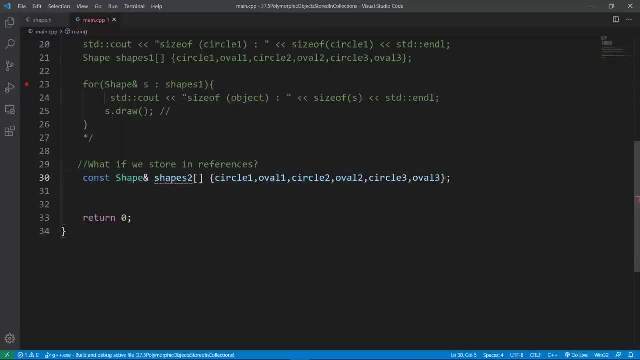 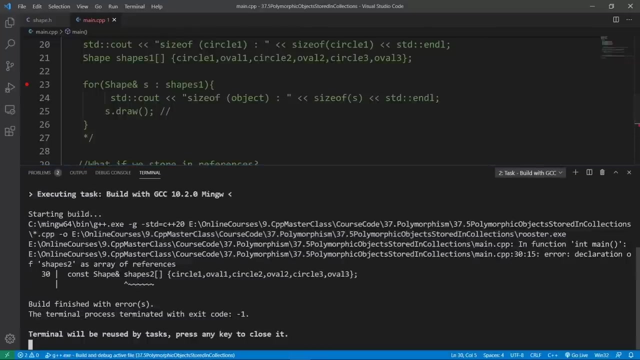 on the types that you can store in your array is that they have to be left assignable and our references are not rest assignable, so this is not going to compile. if we try to build our program, we're going to see that we're going to get weird compiler errors and the build is going to finish with errors. and if we go, 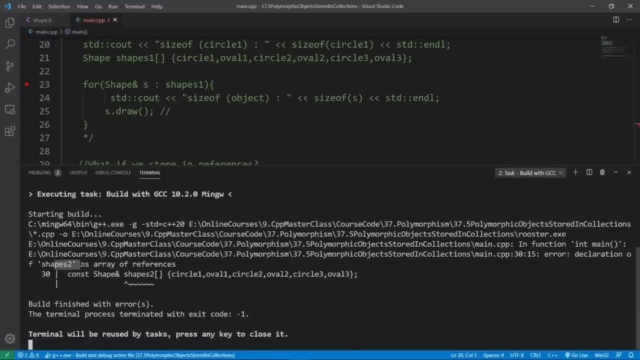 up. we're going to see that declaration of shapes to us array of references, and this is not allowed. you can't have an array of references in C++ and this is the reason why. so we're going to get a compiler error here. okay, so now you know this. but some of you are going to say: what if we go through? 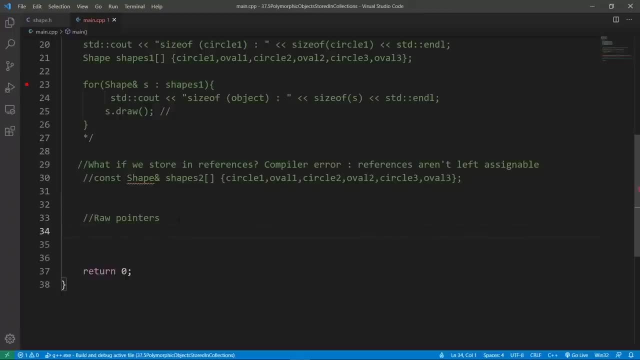 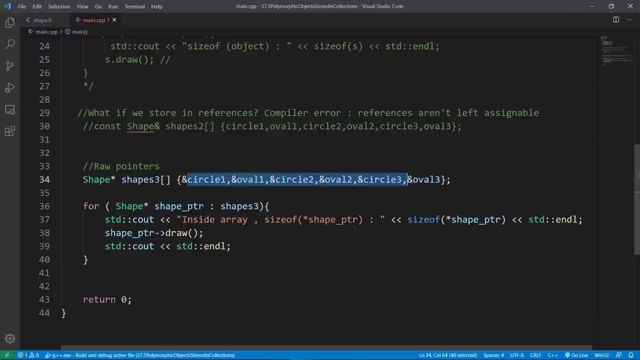 point work, because polymorphism through virtual functions was basically designed to work with base pointers that are managing derived objects, and this is what we have here. so if we look, we're going to be getting polymorphic behavior and if we call our draw method on our pointer, here we're 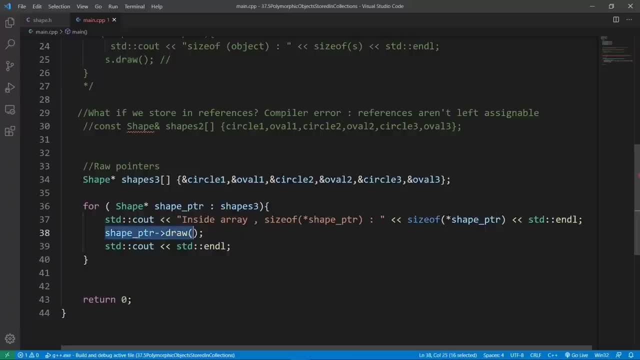 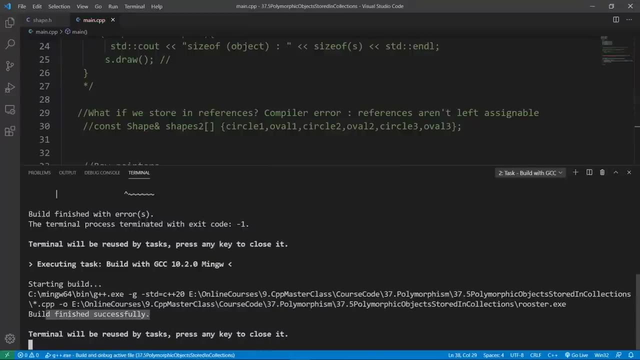 going to get the most specific Joe method called and this is what we want. so we're going to try and build this again and show you that this is going to work. this is going to be good. we can clear and run rooster and we're going to see that we are going. 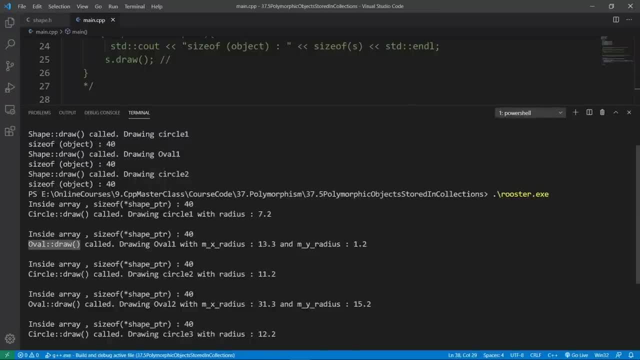 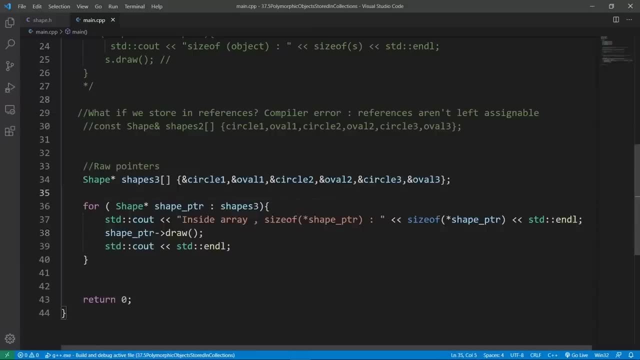 to be looping around and if we call the draw method, we're going to call the over draw method, circle draw method. over draw method, circle draw method. this is basically what we want and we are going through base pointers to really use polymorphism here. this is even going to work if you go through. 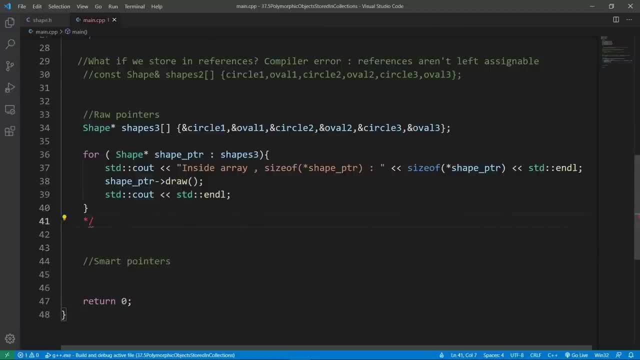 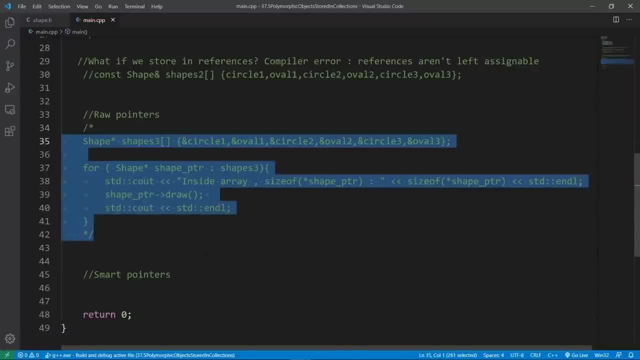 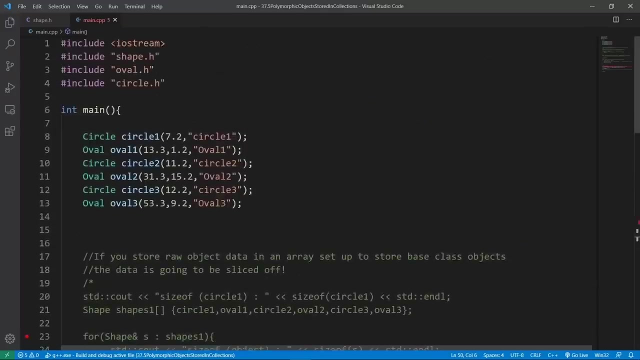 smart pointers. so let's comment this out and set up another example to really drive this home. you can really use any kind of smart pointer. you can use unique pointer or shared pointers. so here we will just be storing again shared pointers, because this is easier to handle, and we're going to head over to the top and include 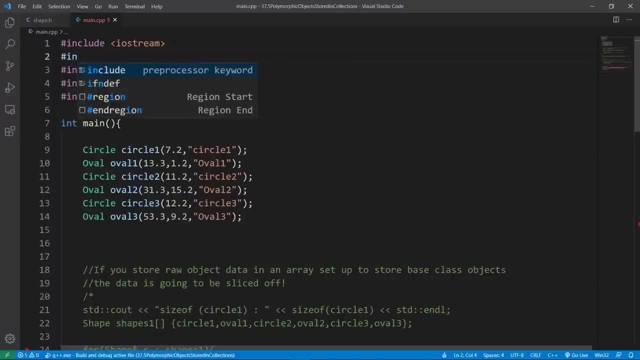 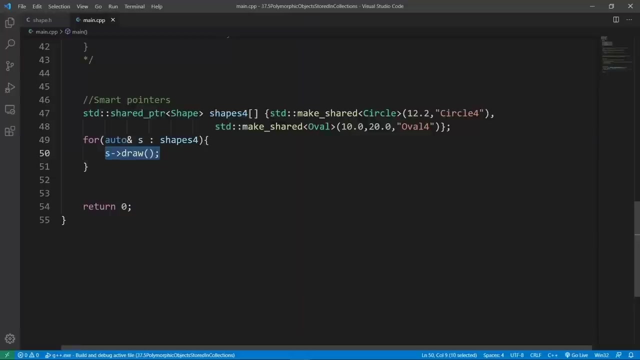 the memory header, if you remember, if you want to use smart pointers in C++, you will have to include the memory header which brings in the data to set up smart pointers in your C++ code. so this is going to look good now and if we build, we're going to get the most specific. 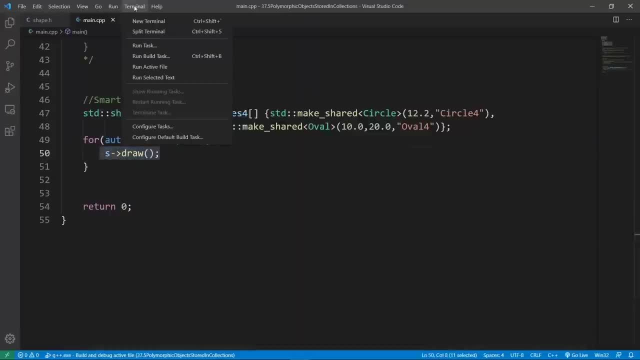 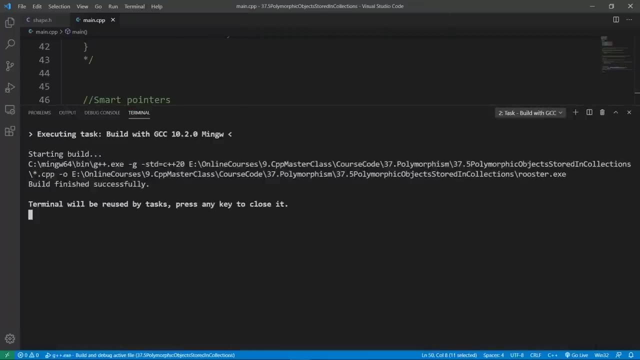 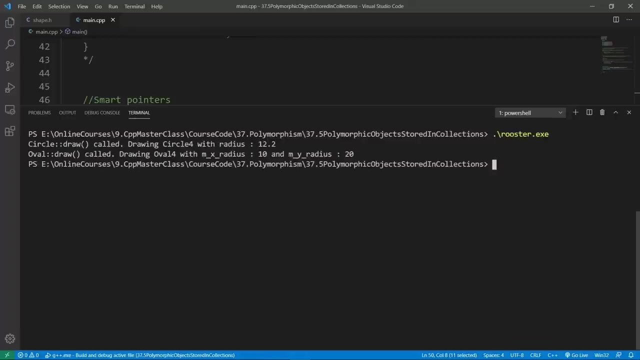 version of our Joe method called through polymorphism, that is, using virtual functions here. so let's build and show you that this is going to work. the book is going to be good, we can clear and run rooster and we are going to get our versions of Joe called the version for. 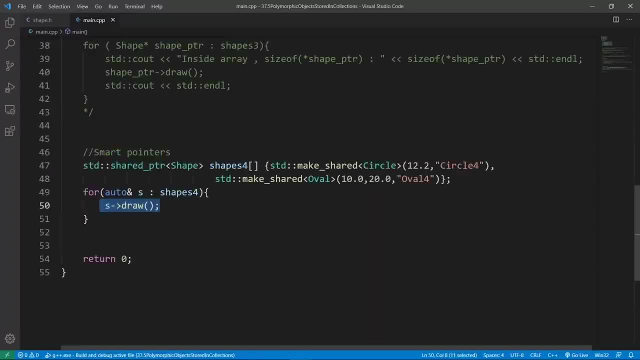 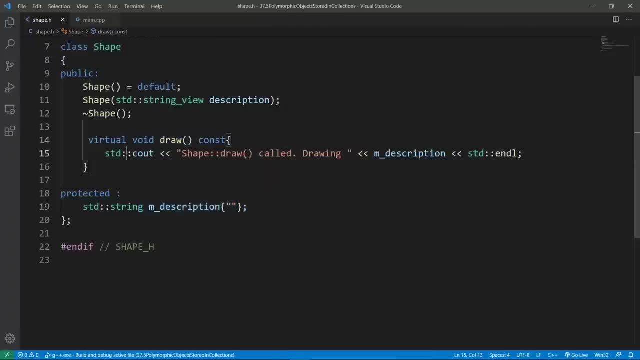 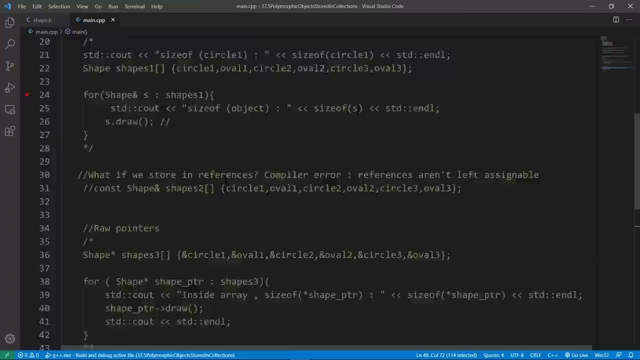 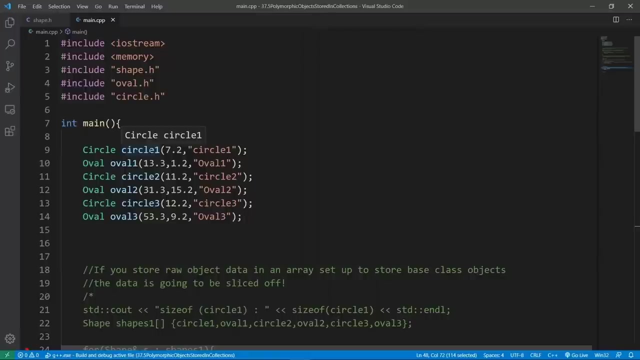 a circle and the version for oval, because we are using base pointers to manage derived objects here and our class inheritance hierarchy is using virtual functions for the draw method here, so this is going to work. this is really all I wanted you to see in this lecture. you should be careful if you try to store derived objects in an array that was designed to. 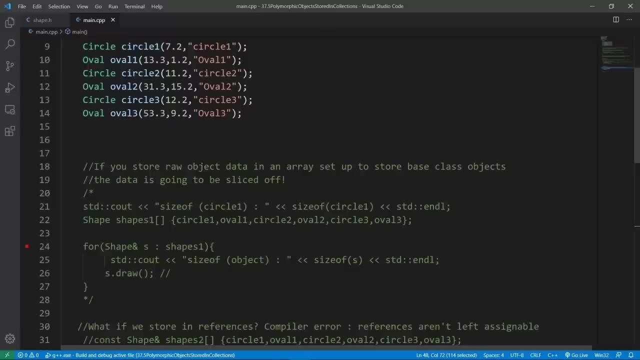 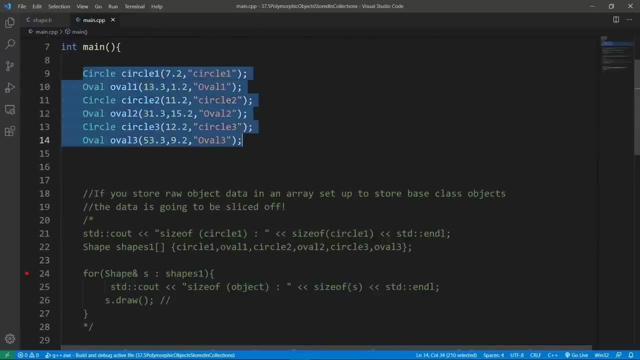 store base class data. if you are using row data, you're going to get slicing and you really need to be aware of this because you want to have derived class information. if you're trying to store any references, this is not even going to compile, because the references 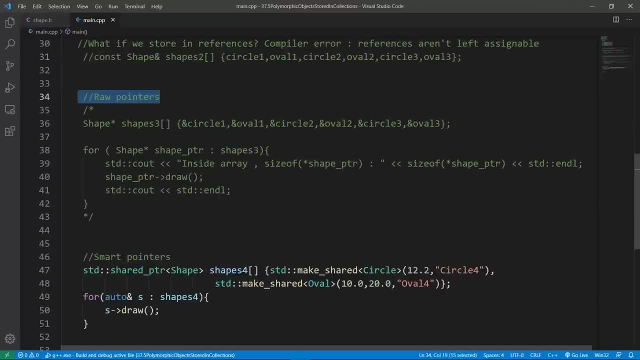 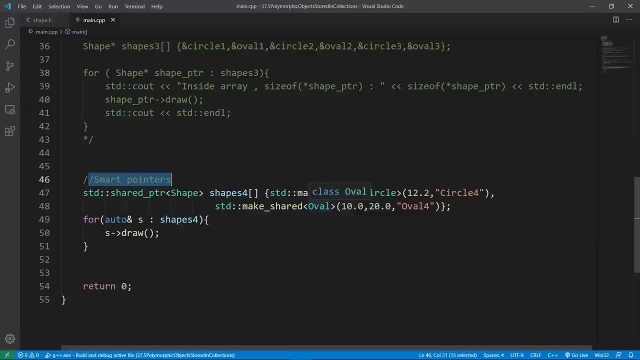 are not left assignable, but this is going to work if you use row pointers or smart pointers, because polymorphism was basically designed to work with base pointers or references that are managing a derived object which uses polymorphism. we are going to stop here in this lecture and 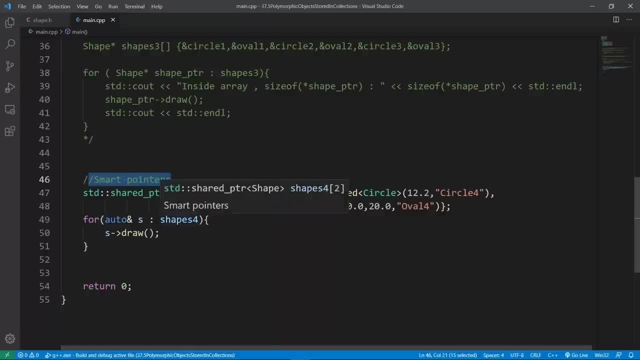 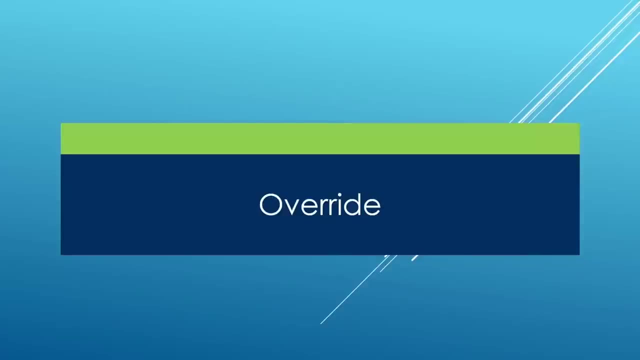 then that's when we're going to learn about the override mechanism in C++. go ahead and finish up here and meet me there. in this lecture we're going to learn about the override specification, a kind of setup you can do to avoid errors in your inheritance hierarchies if you use virtual. 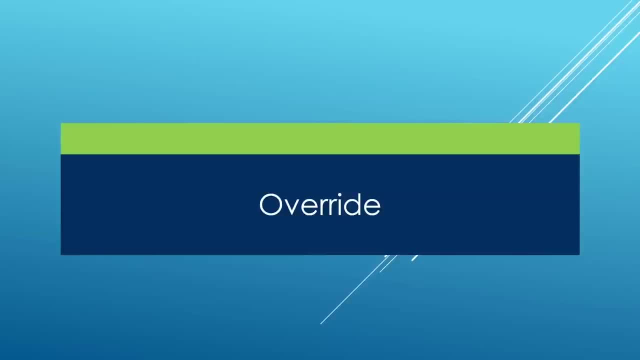 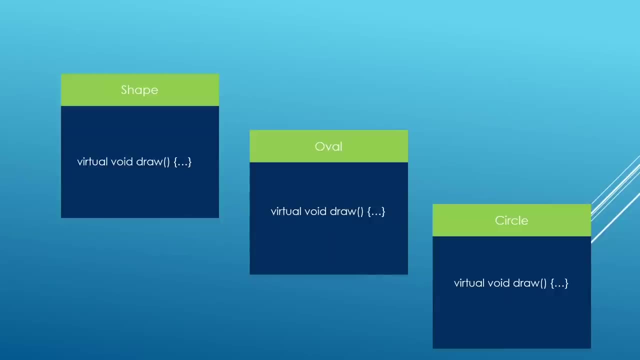 functions to set up polymorphic behavior for your derived objects, and this is something that was set up in C++ to avoid easy to make mistakes. for example, if you have an inheritance hierarchy like this, you might be meaning to set up a draw overrides for what we have in the base class and 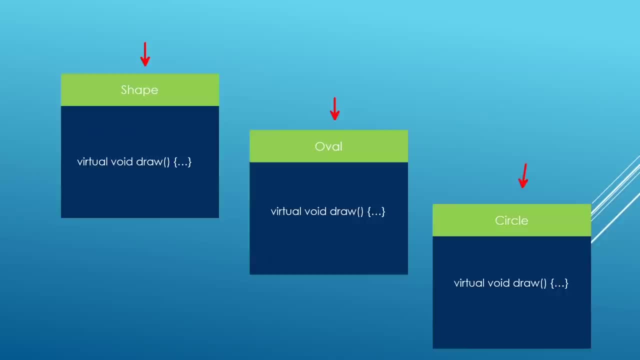 an override is really a most specific method that you have in your derived class to really hide what we had in the base class. for example, the draw method in novel is going to be overriding or hiding what we have in shape and the draw method in circle is going to be overriding or hiding what we have. 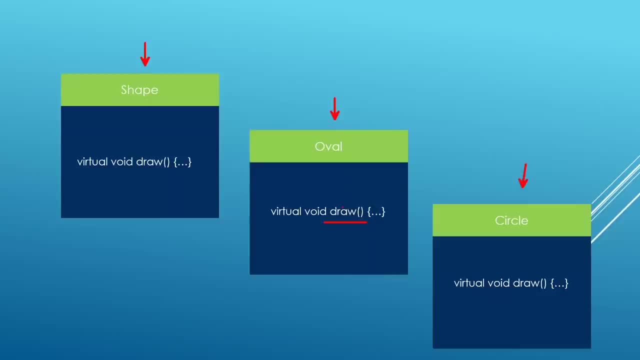 in oval. this is the idea here, but as you set up your overrides, you might make a mistake. for example, you may mean to say, draw and use a W that is in uppercase, and that's going to be bad because what you will be putting in Oval is. 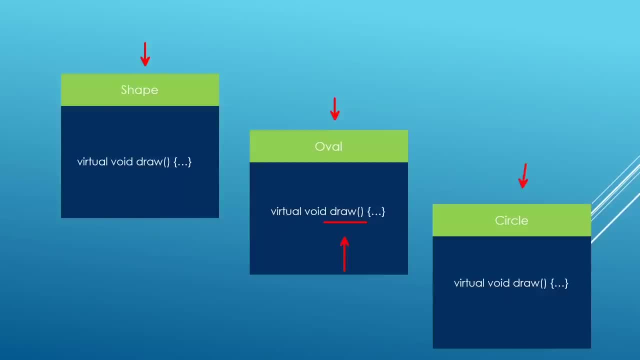 going to be a completely separate method that is different from what we have on the top, and this is going to be really bad. you're not going to get polymorphic behavior for the drug method in tat and word because we are simply not overriding the draw method from shape and 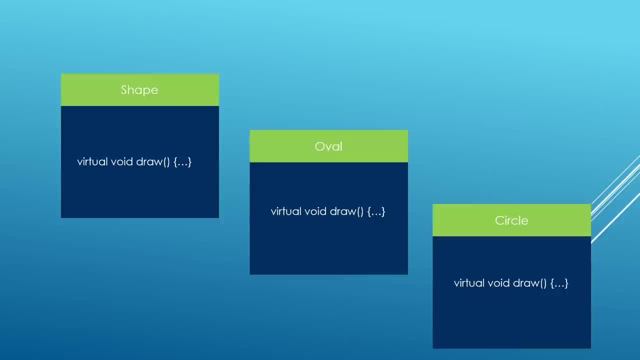 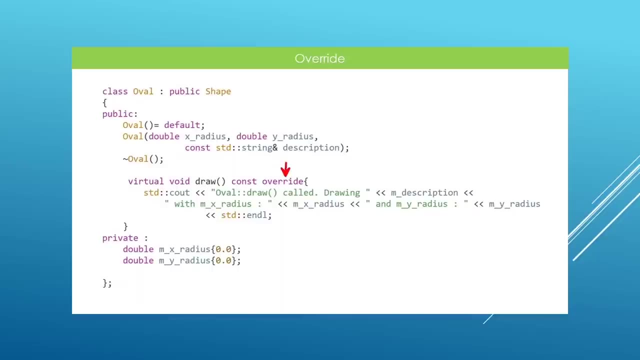 this is going to be bad. so in C++ we can avoid these problems by explicitly specifying that's the method we have in. awful is an override, and we can add this specification after our method header and the c plus plus compiler is going to enforce that. we are actually overriding a method that. 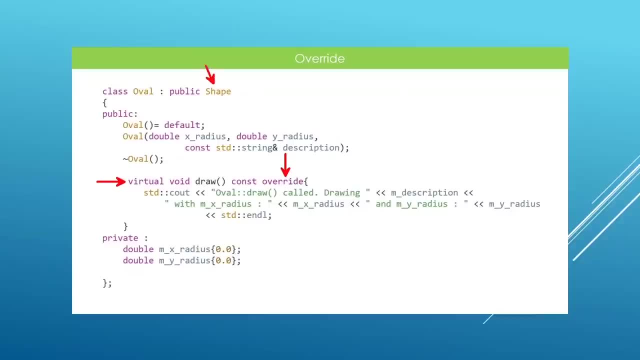 exists in our parents class, which happens to be shape here. if we have no method called draw in the base class, we're going to get a compiler error because we want to be basically overriding any method here. this is going to protect us from problems if we make typos in setting up our 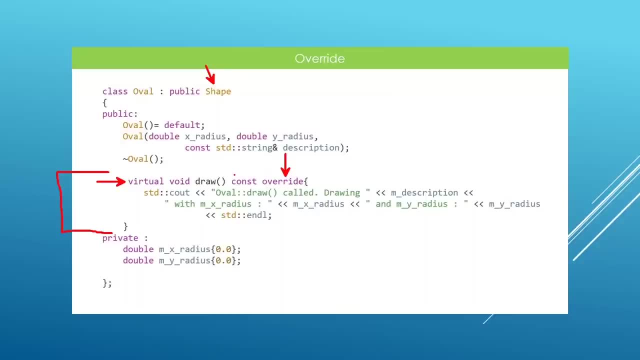 polymorphic methods here. this is the main thing we can achieve with the override specification. now that you know this, we're going to head over to visual studio code and play with this a little more. here we are in our working folder. the current project is override. here we're going to grab the 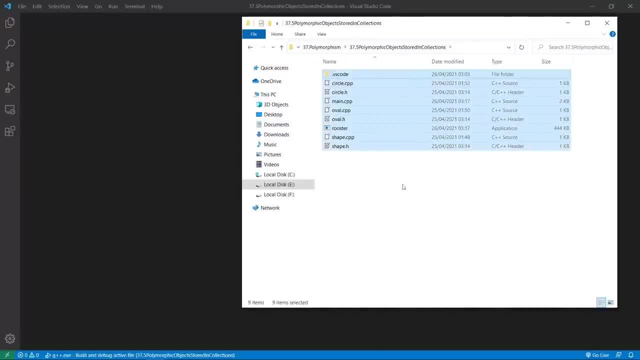 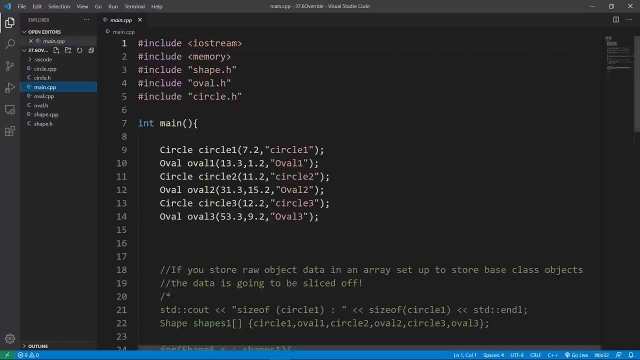 code from the last lecture, because we are basically going to be reusing the same code over and over, welding top of that if we need to do that. so we're going to put in our code and we are going to open this in visual studio code by dragging and dropping here. this is going to give us our code and we 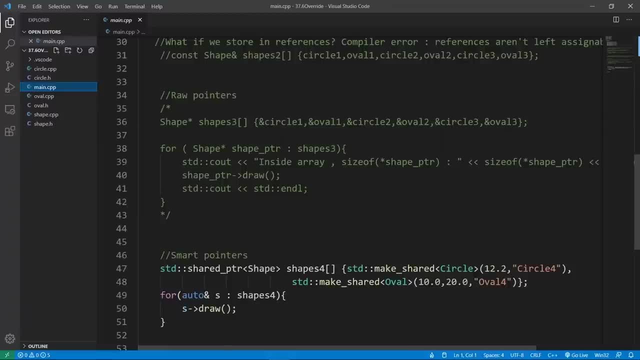 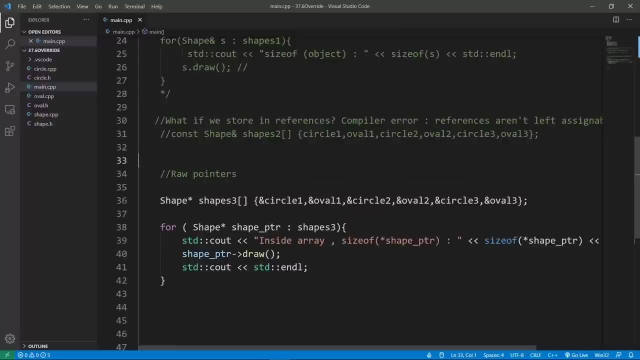 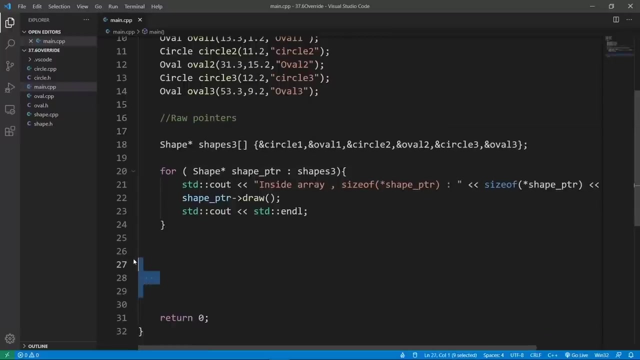 can really do whatever we want with that. i think we can leave in the code that is using the base pointer to manage our derived objects. i think this is going to serve us well enough and we can take out everything else, because that's just going to be confusion. we don't need all this here. this is. 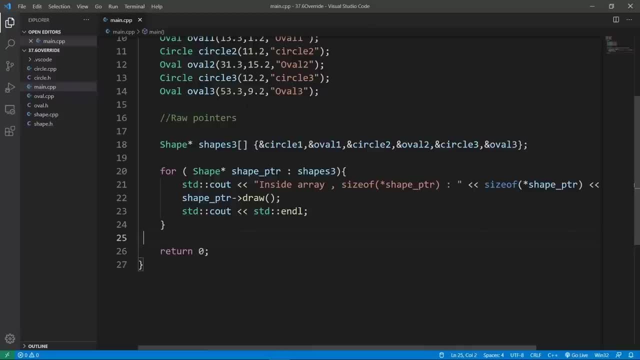 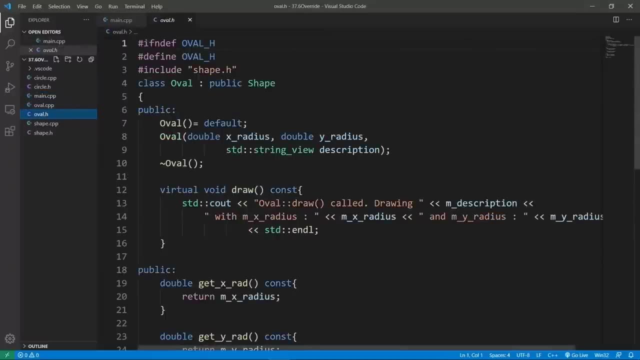 going to be serving us well. now we want to learn about the override keyword and to learn about that we're going to introduce a typo on purpose here. for example, suppose we want to set up a joe override and we use an uppercase letter here for the w keyword. i don't think this is really easy to spot. 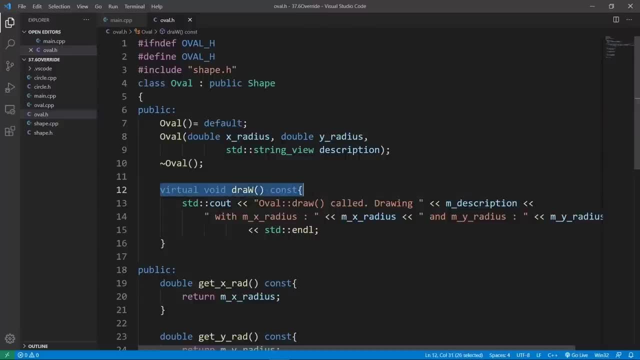 once you've made this mistake and you're not going to be getting any compiler error, because this is something valid, you can set up a compiler completely new method and call it joe and this is going to work, but this will be very hard to spot in your program and the compiler won't protect you, as we just said, if we build our 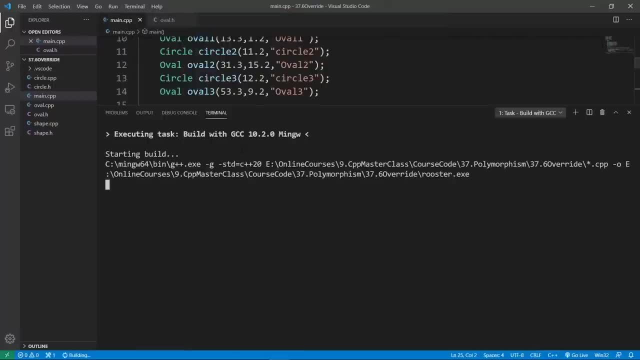 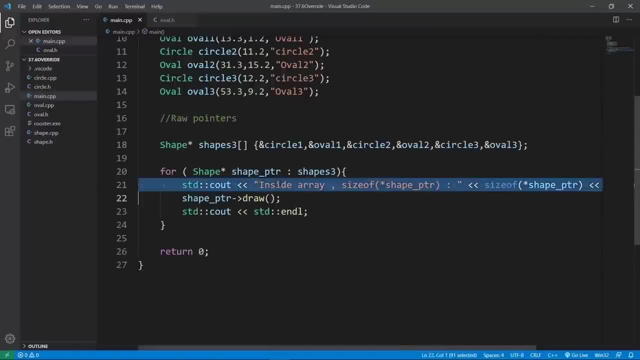 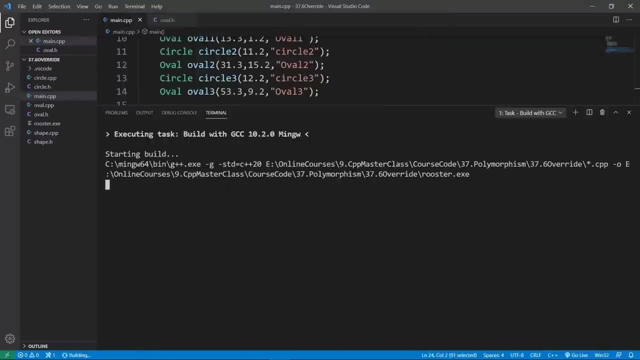 program. you're going to see that it is going to build just fine, so let's pass this through gcc. the build is going to be good, but we want to get to the behavior that we want. i think we can take out this stdc out statement inside our for loop here and we can build again. this is going to be. 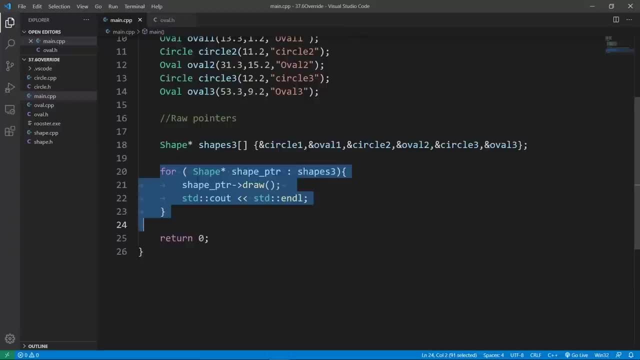 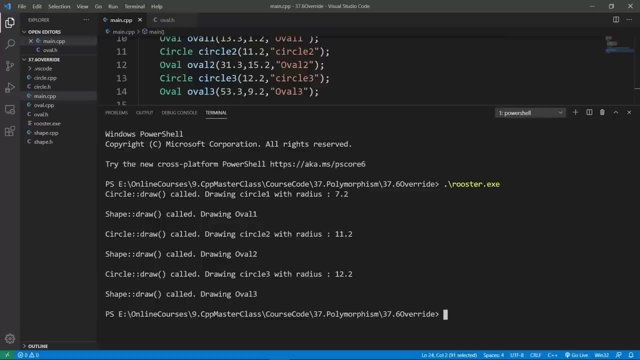 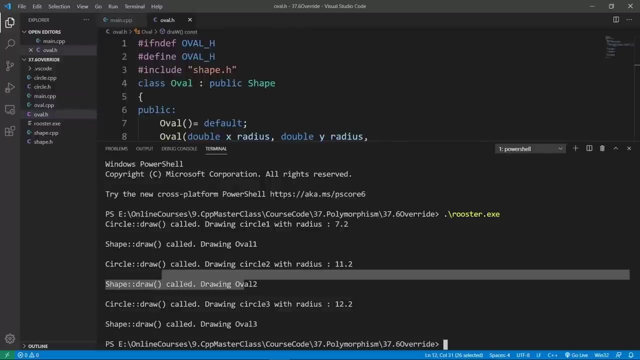 less confusing. okay, so the build is good. we can bring up our powershell window and i'm going to run rooster and see what happens. you're going to see that for a circle, we're going to draw a circle, but for oval, we're going to be drawing shape. so what is happening here? we are overriding our 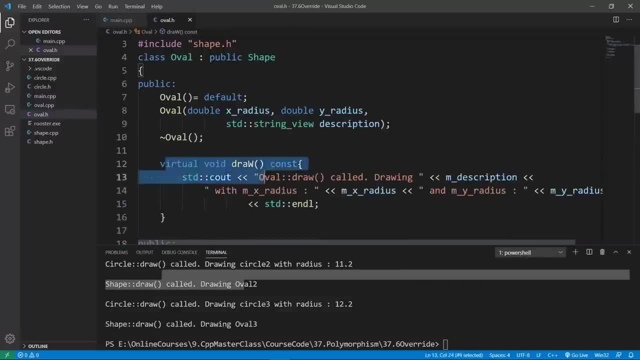 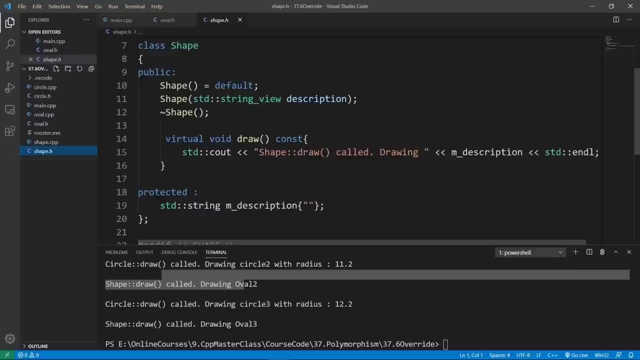 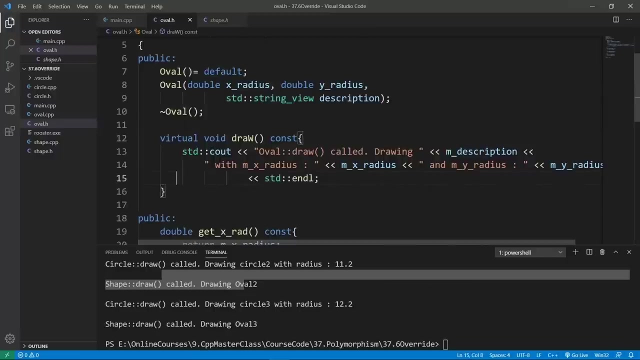 joe method in the oval class. so we should get polymorphic behavior, because this is a virtual function and it is called draw. exactly the same thing like we had in the base class, except we've made a really simple typo here but it is really hard to track and get hold of. we have named our method joe, but the w is in uppercase, so this is: 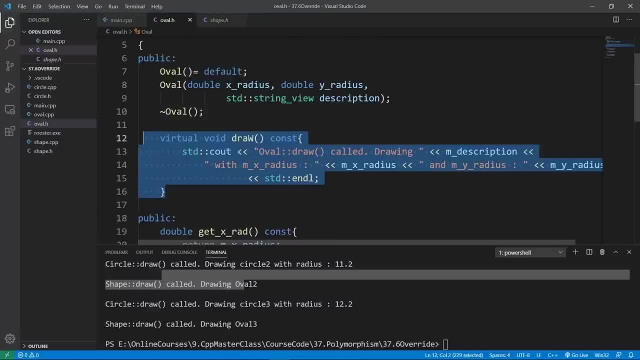 a completely different method than the joe method we originally intended to override in our base class, and this is really hard to get hold of because this is a virtual function and it's called draw. exactly the same thing like we had in the base class, except we've made a really simple typo here. 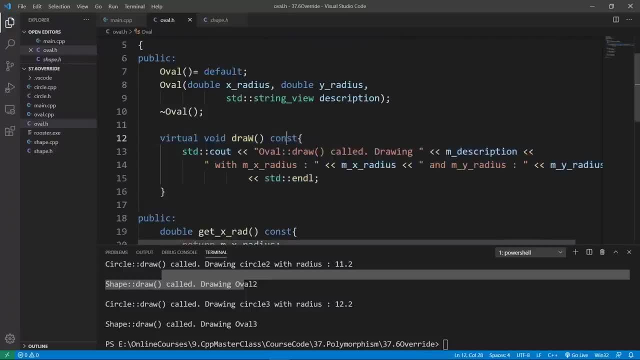 to follow and keep track of. we can protect ourselves by adding the override specification. so if we say override, the compiler is going to help out and make sure that we are actually trying to override a method that exists in the shape class, and if it doesn't exist, we're going 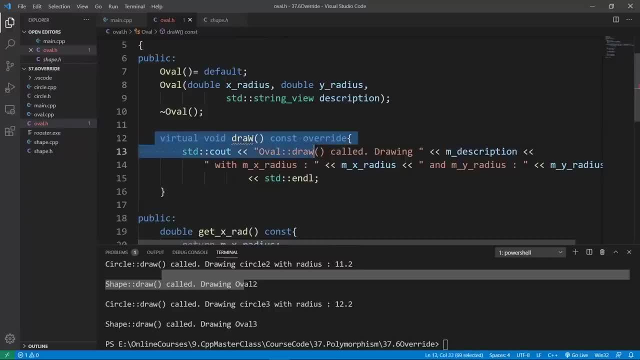 to get a compiler error, then we're going to look at this and really support this mistake here. this is what you can achieve with the override q world and in fact, i do recommend and advise you to use this as an example of what you can do with the override q world, and in fact, i do recommend and advise you to use this. 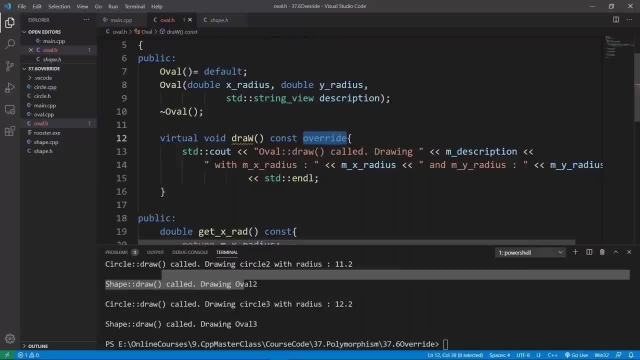 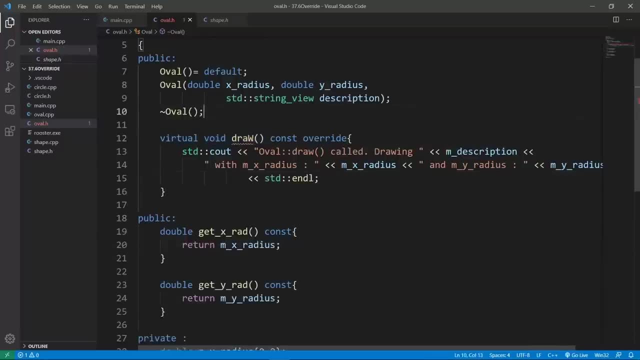 in your inheritance hierarchy if you happen to be using virtual functions, because this is going to save you a lot of time if you make mistakes like this. so we're going to try and run this and show you the compiler error we get. so let's do that. we're going to pass this through gcc the build. 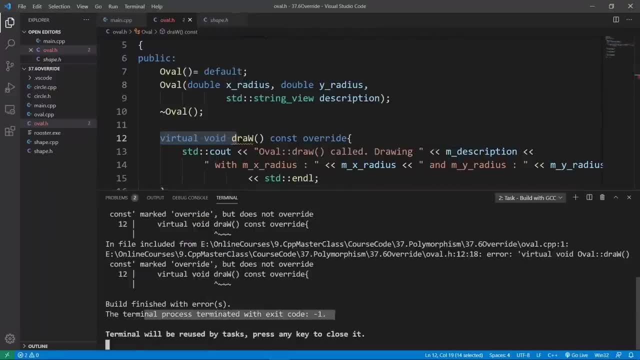 is going to fail as we see here, and we're going to get a compiler error saying error: virtual void overall joe cost marked override but does not override. this is super clear. we are saying we want to override here but we're not overriding any method called joe with an uppercase, because we 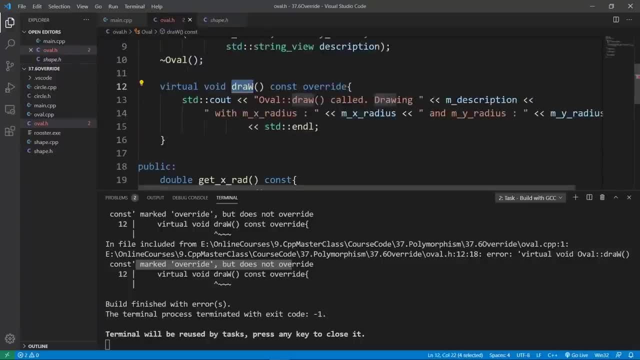 don't have that in shape here. this is the message. once we see the problem, we can correct it. we're going to use in lowercase letter for w, and this is going to work just fine. now we're going to use the same mechanism to protect ourselves from ourselves in circle class. so we're going to 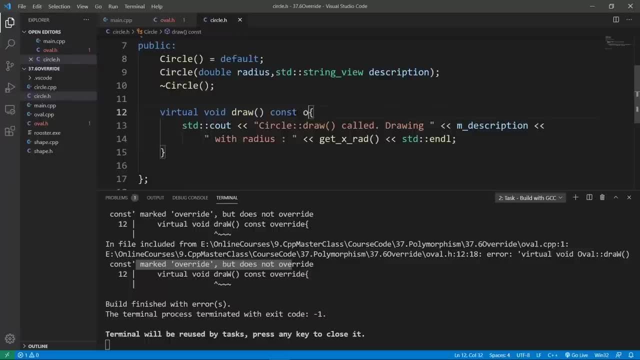 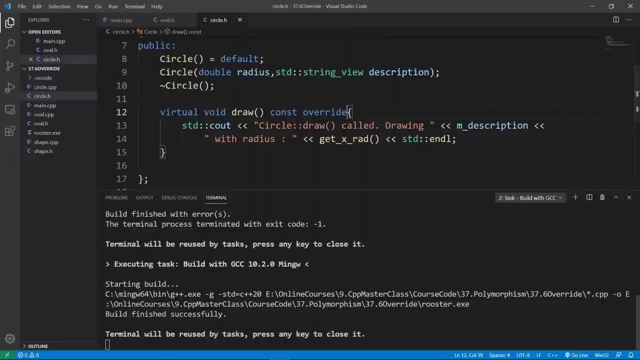 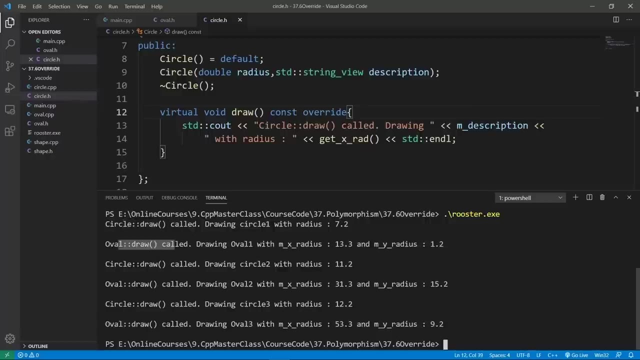 override our draw method. but we're going to say that we want to override explicitly and if we're world now, let's pass this through gcc. this is going to build successfully and if we run our program we're going to get polymorphic behavior. let's do that. you see that circle draw overdraw. 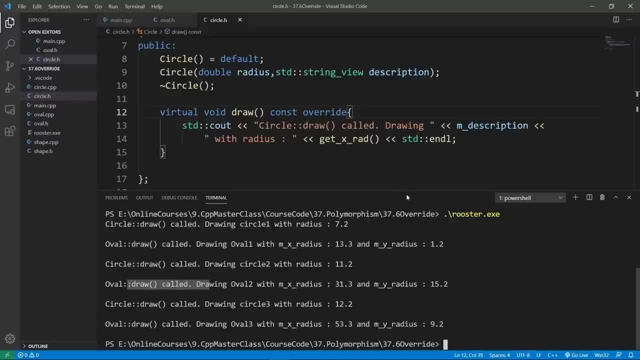 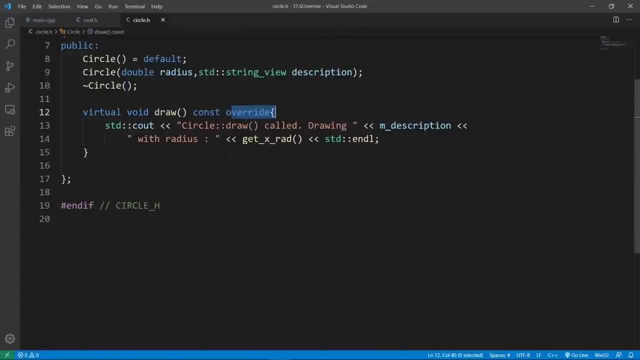 circle: draw overdraw. this is what we expect. this is really cool. this is really all i had to share in this lecture. i hope you found it interesting. use the override keyword in your inheritance hierarchy, because that's going to protect you from easy to make typos. that are really going. 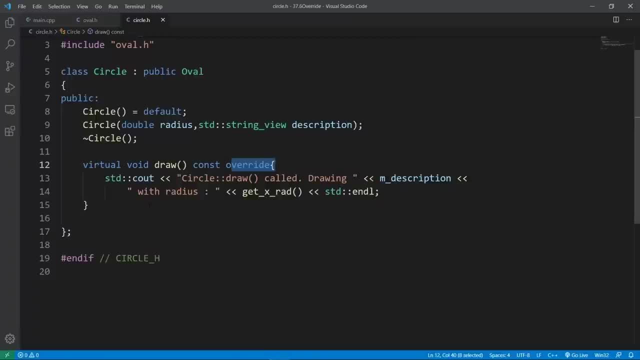 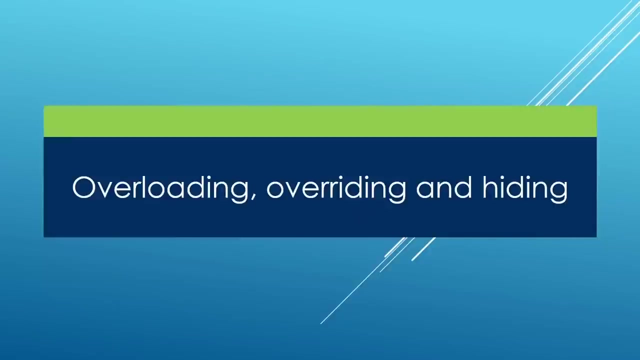 to give you a hard time, otherwise we are going to stop here in this lecture. in the next one we're going to explore the concepts of overriding and hiding in detail. go ahead and finish up here and meet me there. in this lecture we're going to zoom in on overloading, overriding and hiding. we have seen that overriding is a 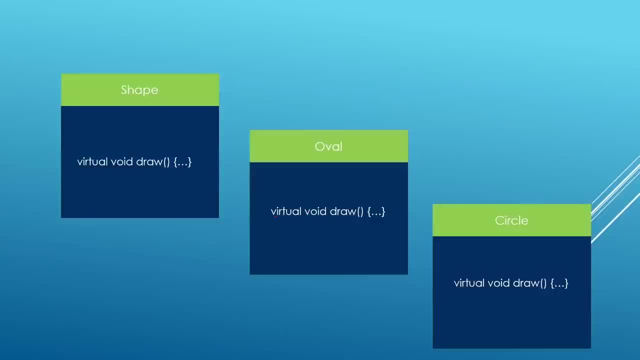 mechanism we have in c plus plus to be able to set up most specific versions of our virtual methods in derived classes. so, for example, the draw method we have in oval is overriding or eclipsing the one we have in shape, and the draw method in circle is overriding or hiding or eclipsing the one we have in oval. this is the concept here. 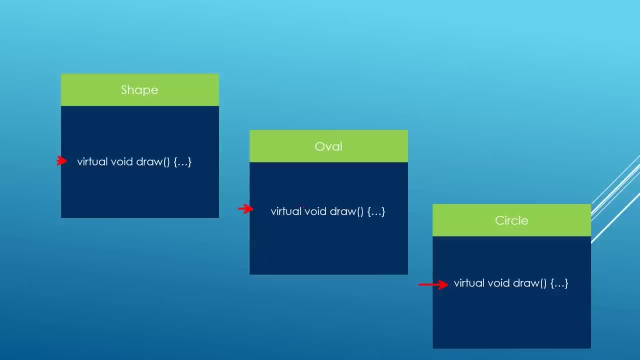 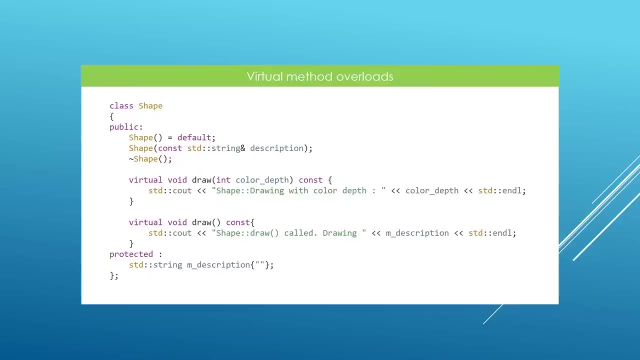 but what happens if we introduce the concept of overloading and mix that up with overriding, as we have seen so far? so suppose we do something like this. this is our shape class. it is going to be going to take a switching structure. we have a few versions of the draw method. we have 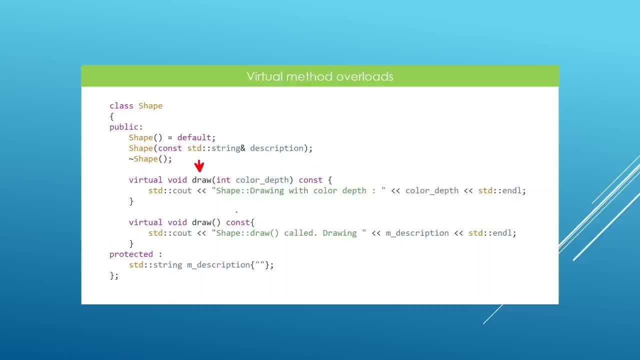 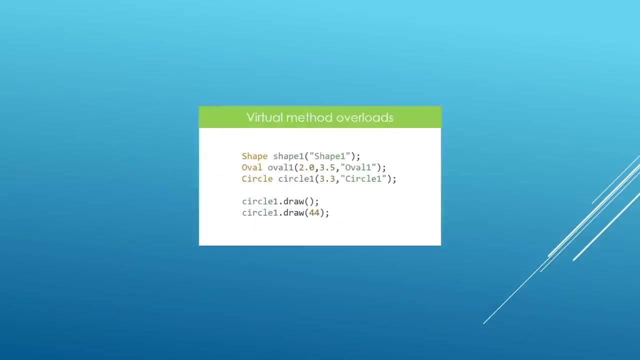 one that takes one parameter- for example, this could be the color that we want to draw our shape with- and another one is not going to take any parameter. and these are two overloads of our virtual method here. so what is going to happen in our derived classes that are going to inherit this virtual? 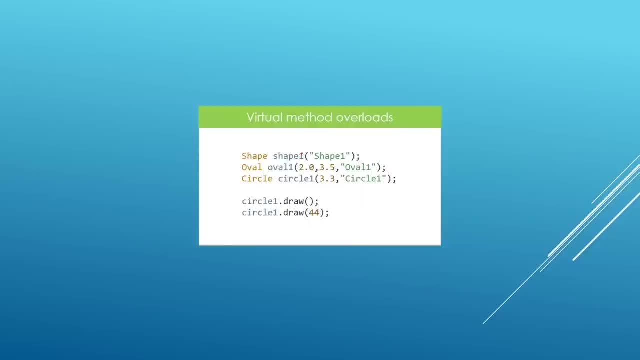 method. so let's look at an example. here we have a simple example that is setting up objects of our and we have a circle object here. if we call the draw method on our must derived class, which is circle, we're going to see that this is going to work. we can draw without a parameter and we can 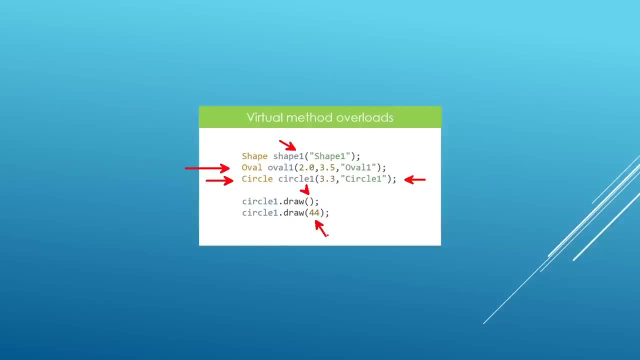 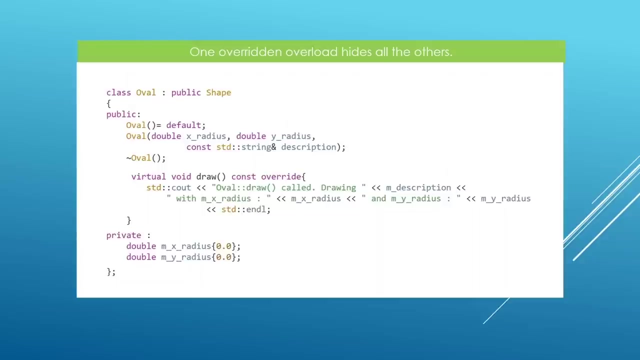 draw with one parameter, which is going to be our color depth. this is going to work just fine. we will be reusing our inherited method from the shape class, and this is really cool. but what happens if you override this method in our over class? suppose we hijack the inheriting process? 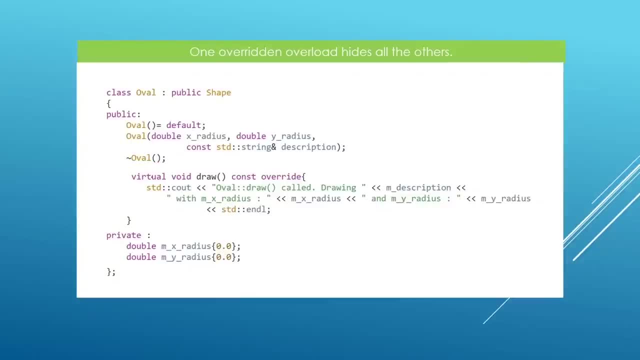 and set up another draw method in our over class and we only override the overload. that doesn't take any parameter. we can do something like this, but the moment you do this, this is going to only override this method and it is going to hide all the other draw methods that we had in our base. 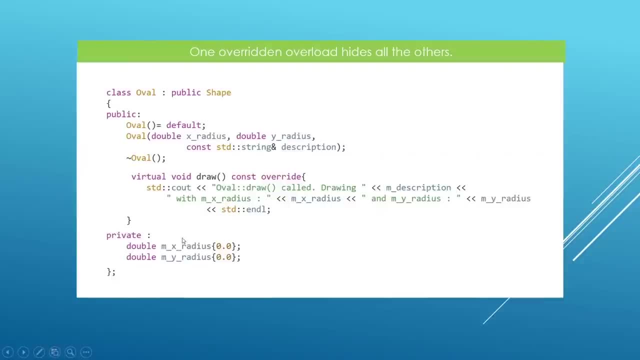 class, which is shape here, and this is something i want you to know. so once you override a single overload of your virtual functions, all the other overloads are going to be hidden and they won't be usable anymore by downstream inheriting classes if you want all the overloads to be available to. 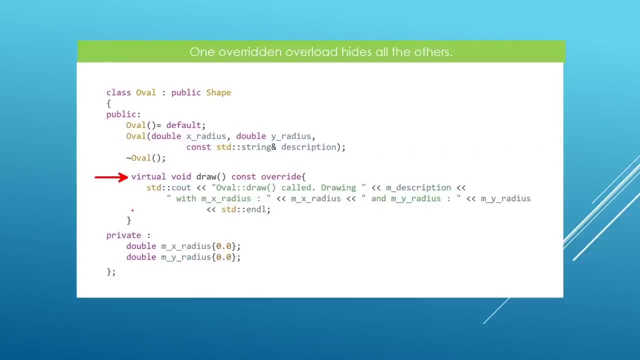 downstream inheriting classes, you have no choice but to explicitly override each of them, and that's how it's going to work. so if we look at the example of the example here, we're going to see that the draw call without a parameter is going to work, because 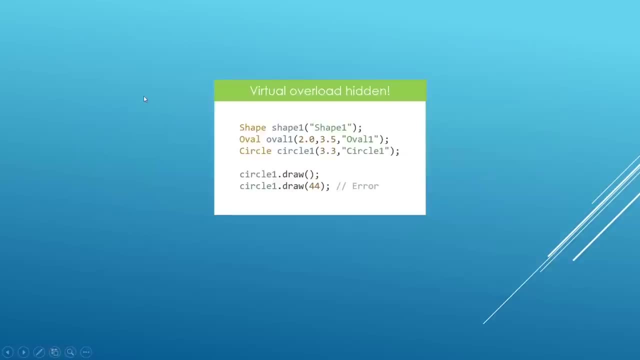 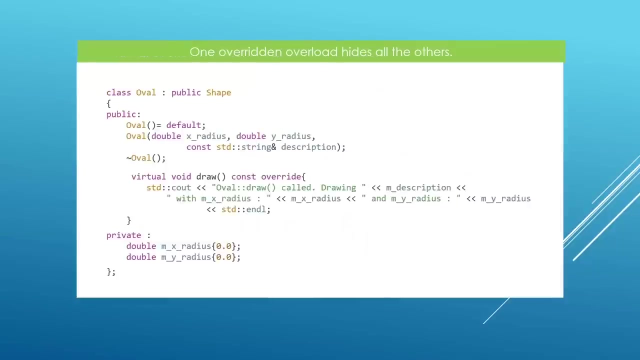 this is overridden in our over class, but if we call the one which takes a parameter, this is going to be hidden at the over level and we won't have access to that in circle, and if we're trying to call this, we're going to get a compiler error again. the message is: if you override one overload. 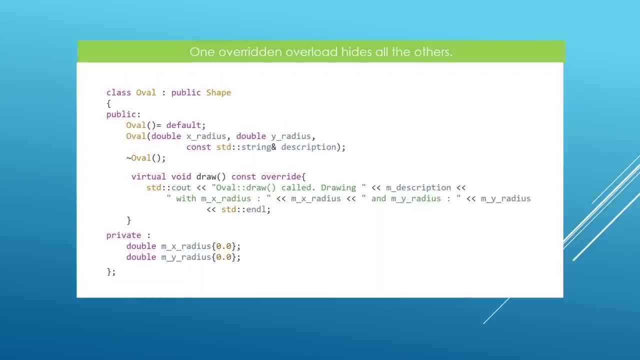 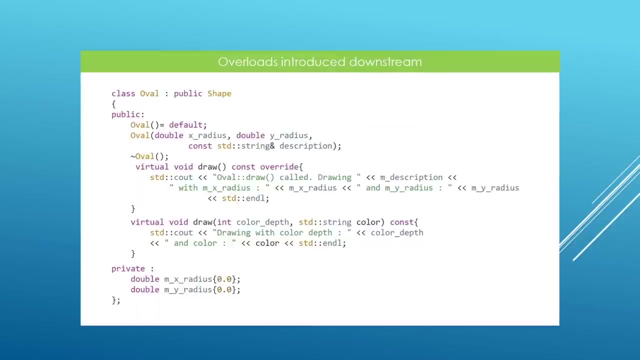 of your virtual functions in the base class. all the other ones are going to be hidden, and you have no choice but to explicitly override them for them to be available and usable in downstream classes. this is the message i want to convey here. okay, so now we know this, but what if we set up another overload downstream? for example, what if we go in? 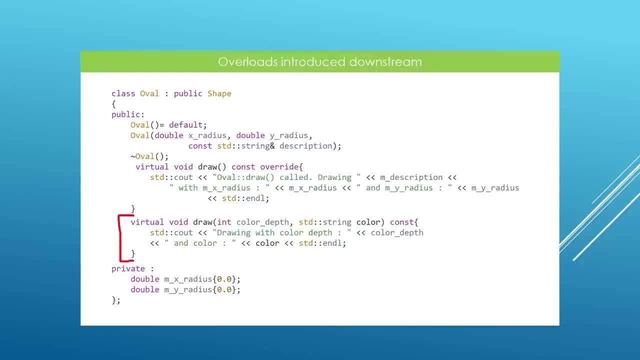 our oval class and set up another overload which is going to have two parameters. for example, we might have the color depth and the color here that we want to go with, okay, so one thing you should know is that this, this method, is not going to participate in. 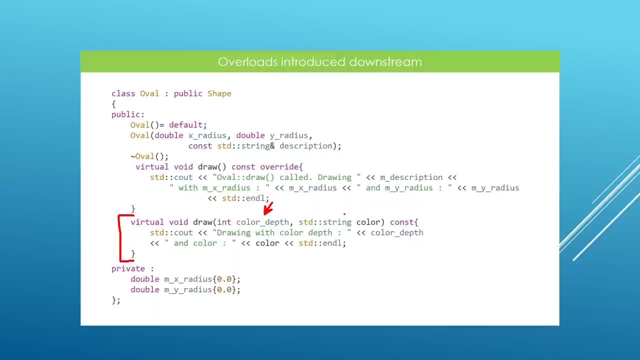 shape polymorphism, and what i mean is that if we go through a base pointer or reference to manage derived objects, we can't really call this method with shape polymorphism. so if we go through our shape pointer or reference, we won't be really able to call this method. if we're trying to call it, we 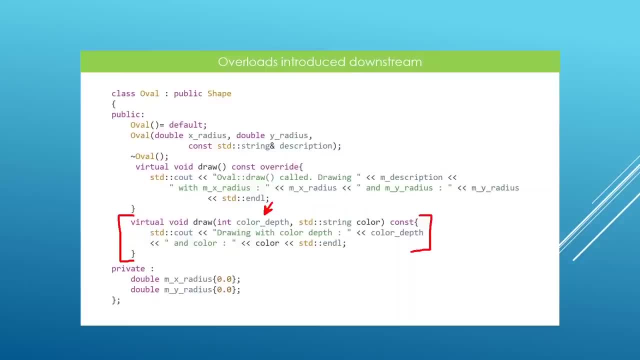 will get a compiler error. the reason is: this method is not known to the shape class. that's why it's not going to participate in shape polymorphism. the only methods that are going to participate in shape polymorphism are the methods that are declared in the base class, and they are 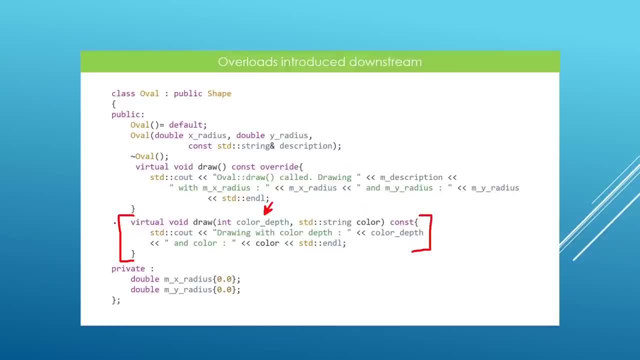 virtual. this is the condition here, and if you violate this condition in any way, shape polymorphism or base class polymorphism, in this case, is not going to work and you will get a compiler error. so if you're trying to do something like this and you want to call your draw method with two, 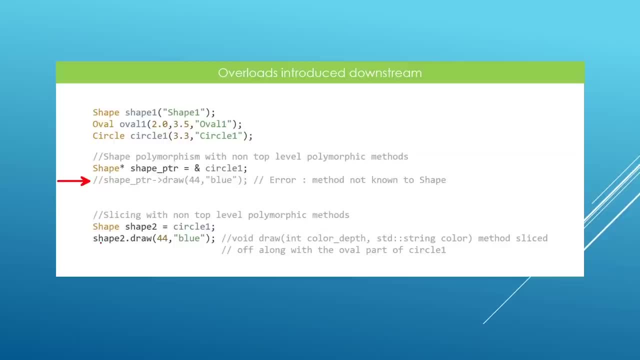 parameters, you're going to get a biometric error and you're going to get a biometric error and you're going to get a biometric compiler errors and this is not going to work. another thing i want you to see is that if you assign a derived object to a base object, your derived virtual functions are. 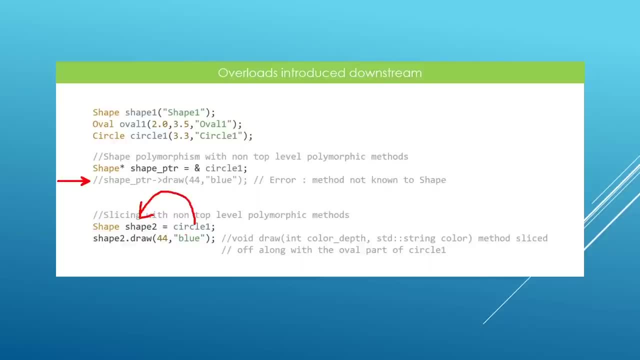 going to be wiped out as part of the slicing that we have learned about already. so the circle port is going to be wiped out, the oval part is going to be sliced off and the draw method is going to go with our oval part and we will only be left with the shape port. 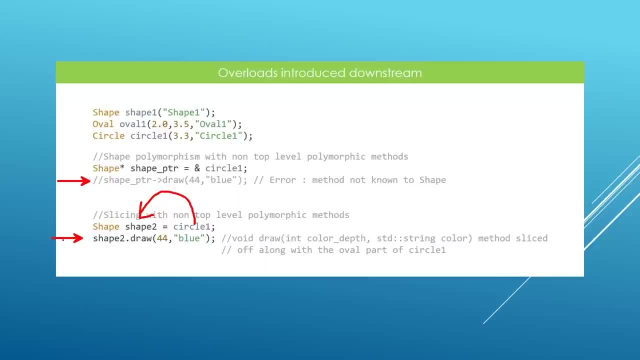 and if we try to call this method here, we will get a compiler error because it's no longer available. it's been sliced off. this is really what i want you to see here. now that we know this, we're going to head over to visual studio code and play with this a little more. here we are in our working. 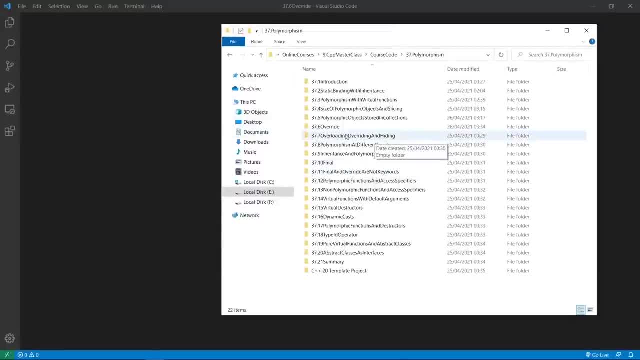 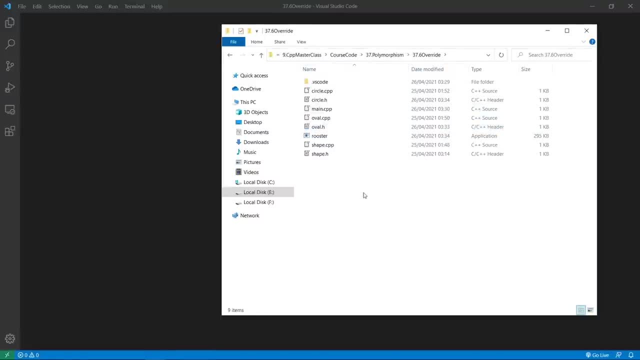 folder. the current project is overloading, overriding and hiding. we want to explore these concepts in a little more detail. we're going to grab the code from the last lecture because that's going to be a good starting point. we're going to take out the binary. we don't want. 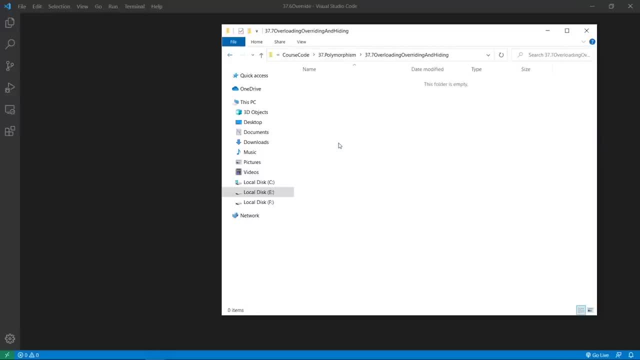 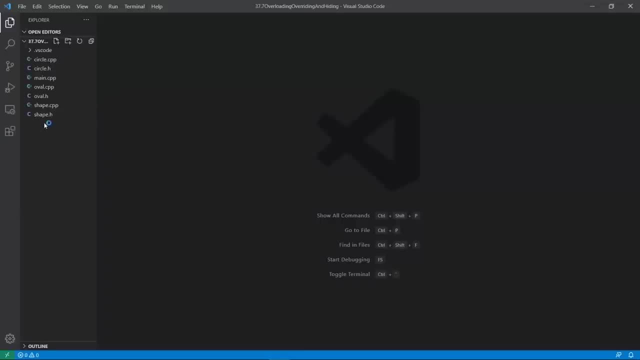 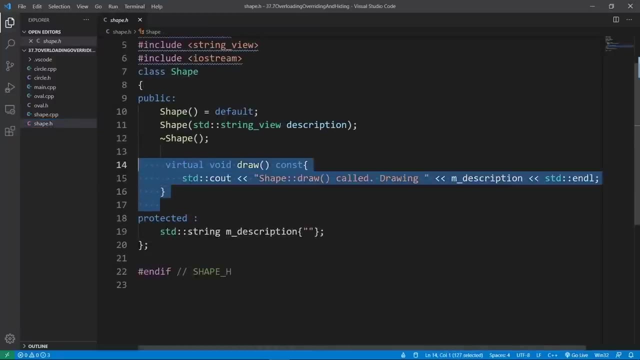 that and we're going to copy and we're going to put that in our current project here. this is going to do and we are going to open this in visual studio code pretty quick by dragging and dropping here and we're going to see that we have a bunch of virtual functions here. just have the joe version. 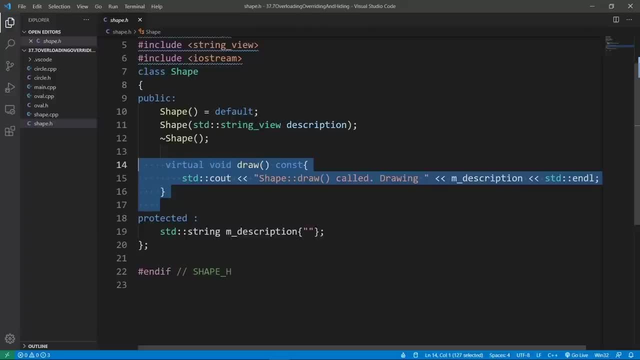 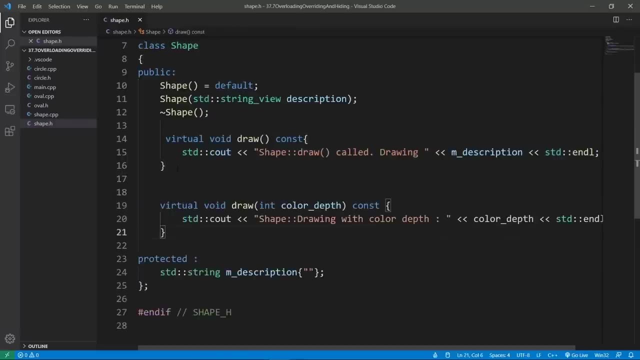 but we can set up an overload of this draw method here. this is what we want to do, so i am going to go below here and set up an overload of this method. this is going to be taking the color depth parameter and we want to see how usable this is downstream, so we're going to go down in the main. 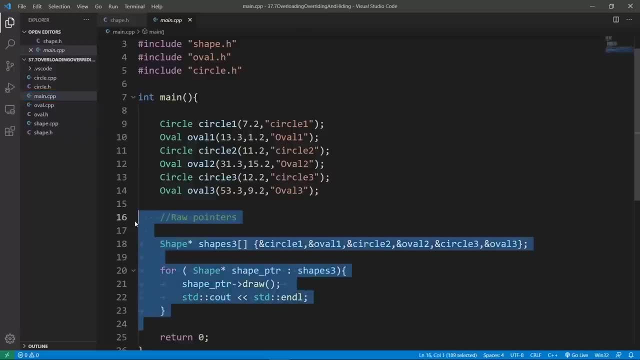 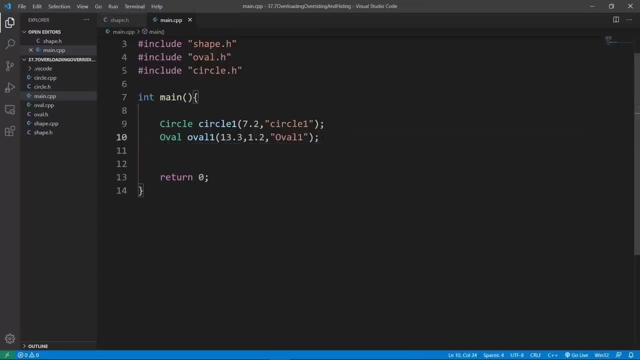 cpp function and take out what we don't need here. we really need a bunch of objects. we can set up circle one and oval one and we will see that we can call these methods. we're going to say, circle one, draw, without a parameter and we're going to say circle one, draw and pass n 44 as our parameter. 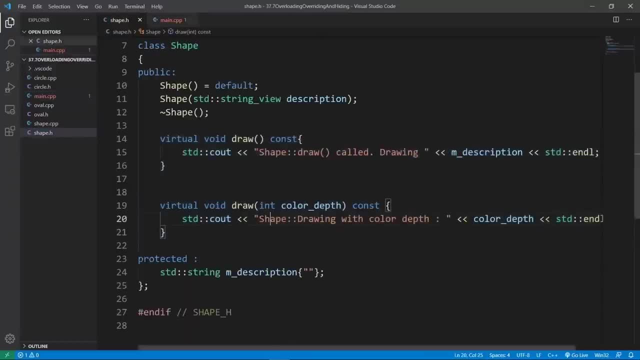 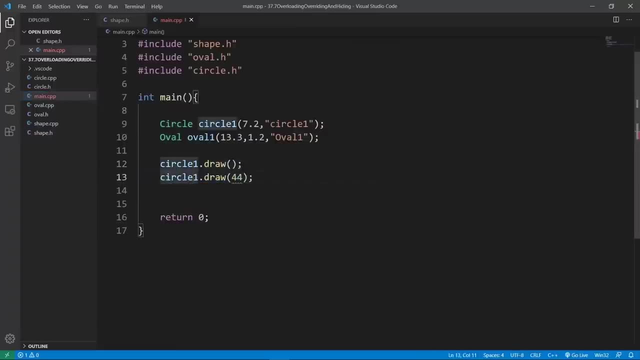 and let's go back and make sure that we have a our overload and this is going to be taking the color depth and let's try and build our program, because we have a squiggly line here. let's see if it is just a visual studio code: playing games. 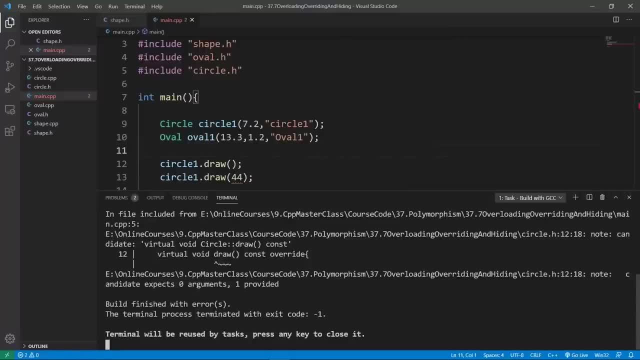 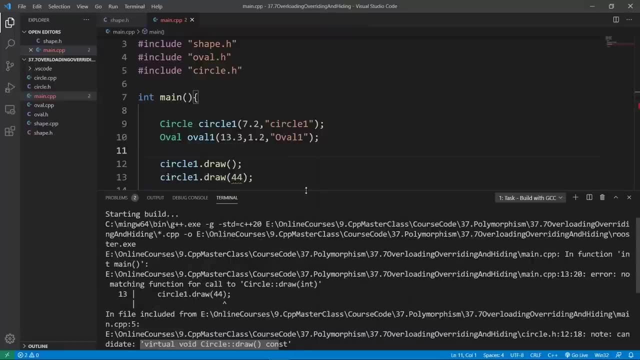 with us. we're going to pass this through gcc and we will have a compiler error here. so what is going on? candidates: virtual draw cost. let's go up and see what kind of problem we have here. ah, this is the concept we just talked about in the slides. we are setting up our 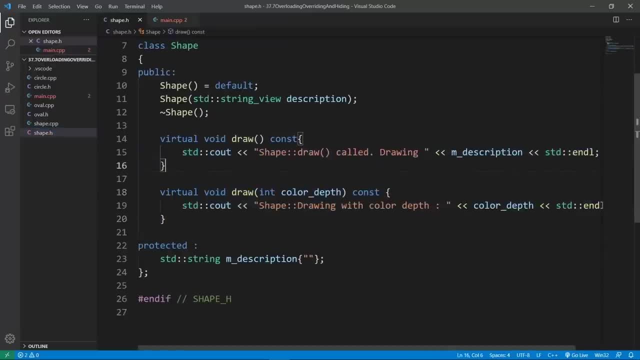 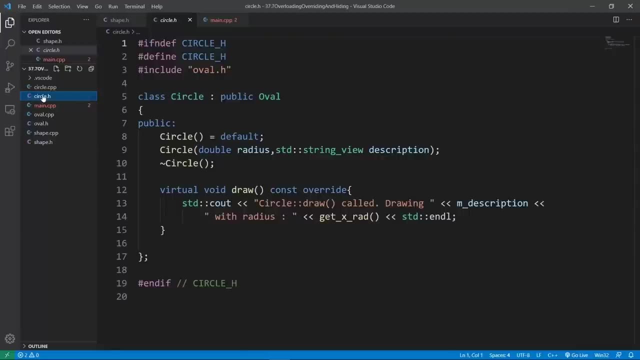 overloads here, but this is being eclipsed by the overloads that we are setting up in oval. you see, we have a draw override and this is also being eclipsed by the override we have in our circle class here if we want the two overloads we have from shape to be available. 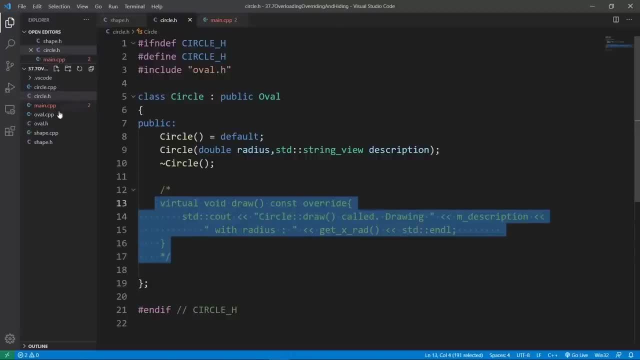 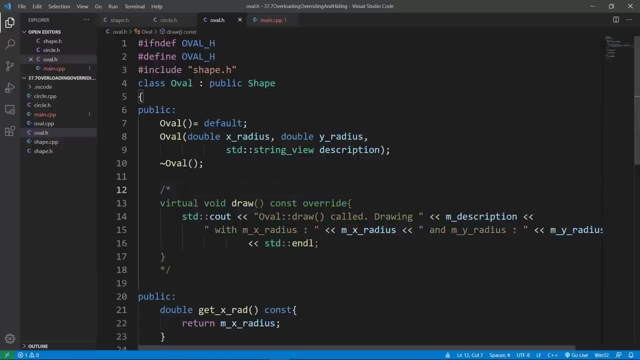 we can comment out the overrides we have both in circle and oval. let's do that and that's going to be available and usable. so let's do that. this is a really good learning opportunity and now, if we go in main cpp, we're going to see that this is going to become available. 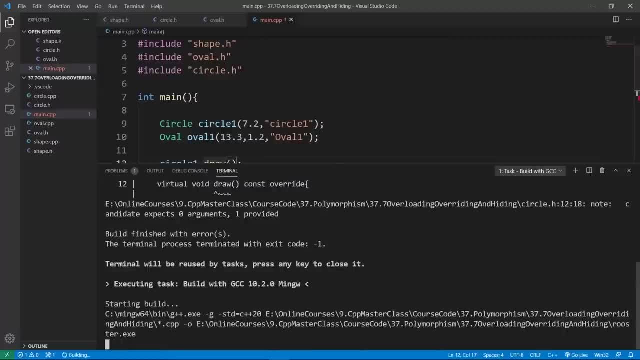 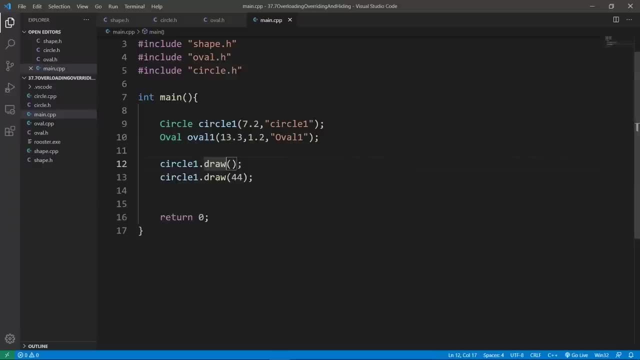 so we can upload this with gcc again to bring visual studio code up to date. and you see, the build is good and our methods are usable, even from derived classes. so, for example, we can also set up a novel object, let's say over one, and say: draw, this is going to work if we say over one. 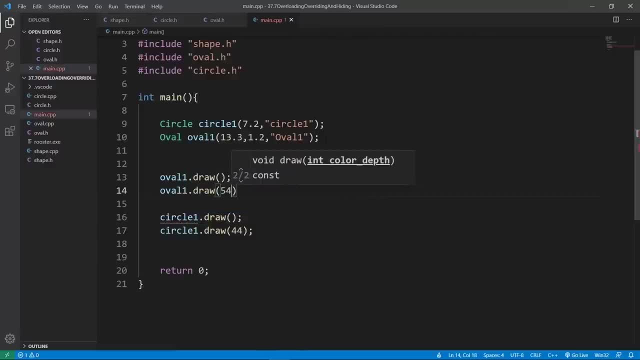 draw and pass in a parameter that's put in 54, for example, and then we can also set up a render function and say: run this is going to do. you're going to see that this is going to be accepted by visual studio code and if we build and run this program, 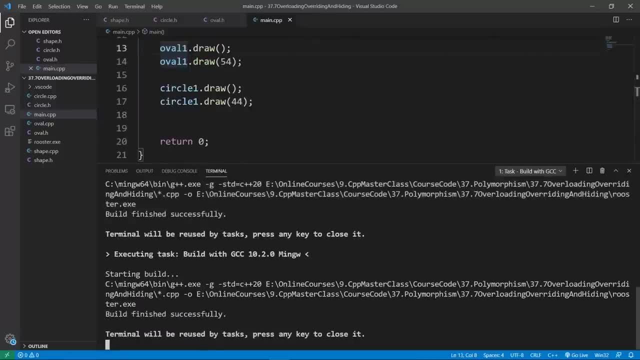 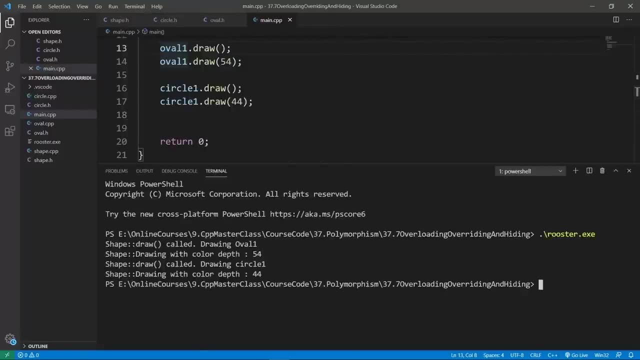 it is going to build. it is going to be calling the inherited functions in oval and circle. here the build is good. we can kill our terminal here and bring up a powershell window we can use to run our program. we're going to see that we call shape draw and shape draw, because these are 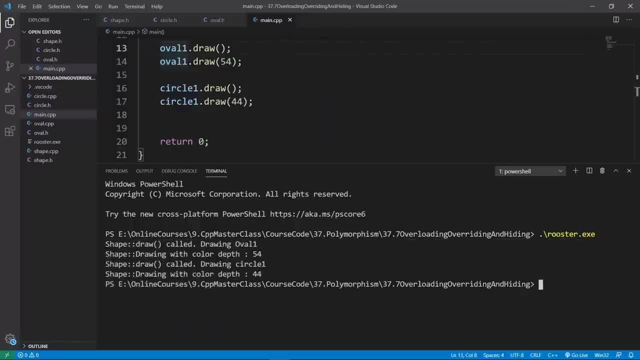 the shape class. that's why we are saying: shape, draw here. and we're going to be drawing our oval and drawing with a color depth. we're going to be drawing the circle and drawing with a color depth here. this is the message i want to convey, but the moment we override these methods in any, 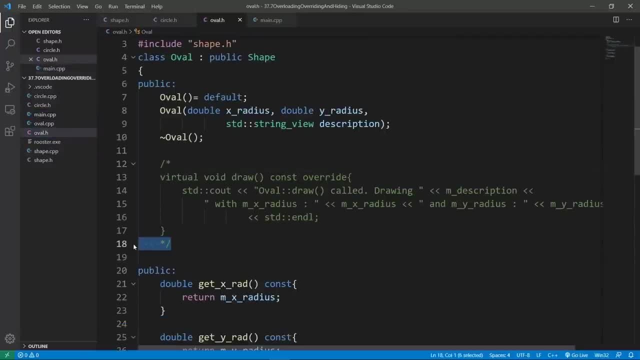 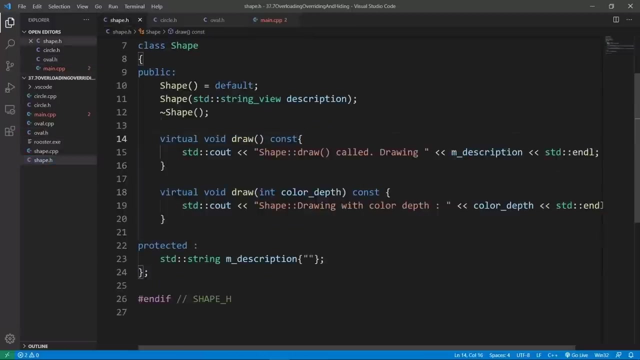 downstream class. for example, if we go in our oval class and uncomment out the override for the draw method, notice that we are just overriding a single overload. again, if we go back to our shape class, we have an overload that doesn't take any parameter. we also have an overload which is: 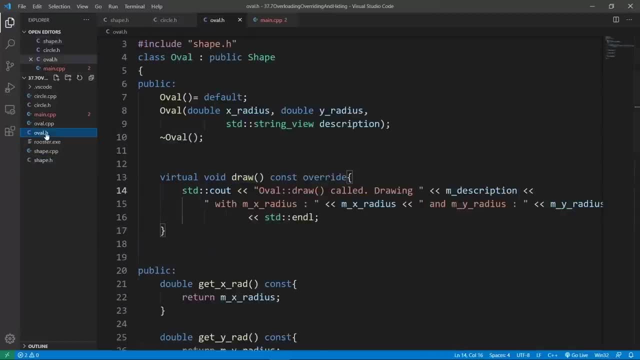 going to take one parameter in oval. we are just going to override the overload that doesn't take any parameter. but this is going to hide all the other overloads we had for the draw method here and this is the only overload that is going to be available in downstream. 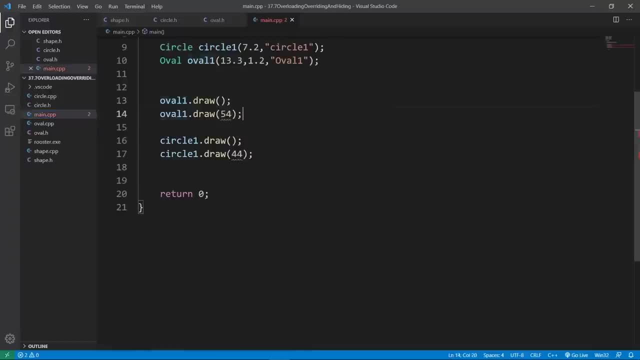 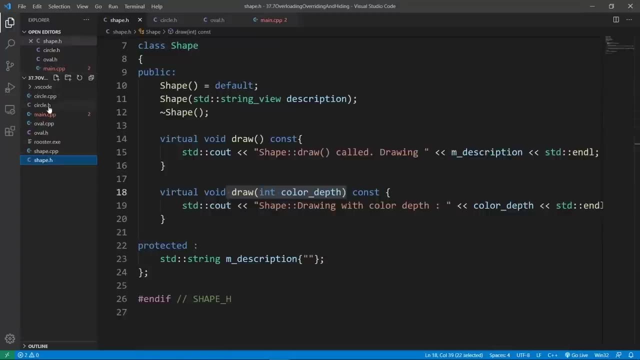 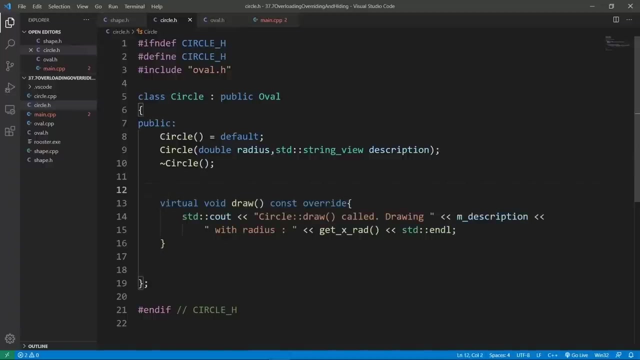 і classes. so if we go back in main, we're going to see that the one with a parameter is not going to work and we're going to get a bunch of compiler errors. this is going to be the case even in circle. if we uncomment this guy, the others are going to be eclipsed again. the other one we have is just: 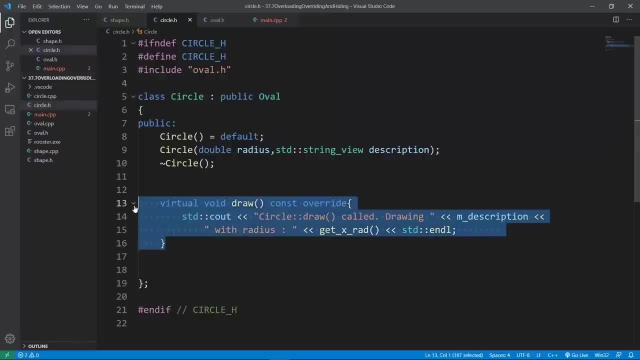 the one with one parameter, but this is going to stay true even if you have a hundred overloads. all the others are not going to be available if you happen to only override one of the overloads. in other words, the other overloads are going to be hidden by this one override that you are putting. 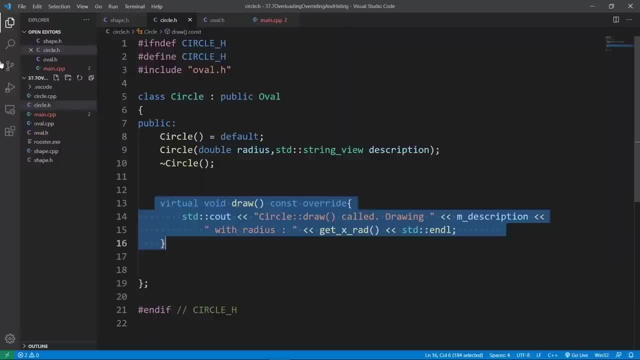 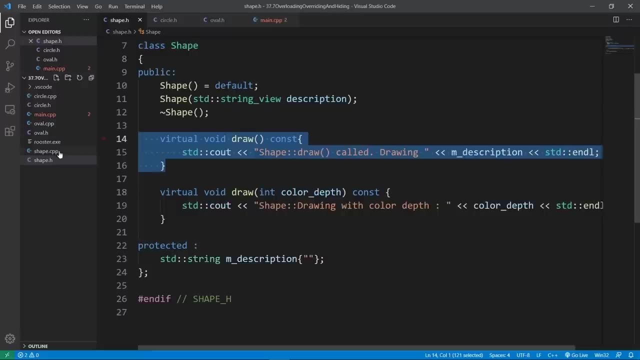 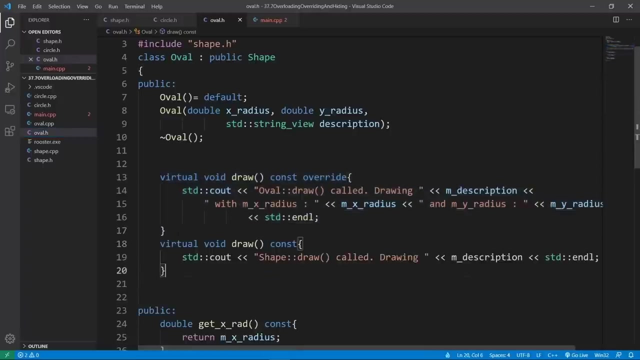 in your inheritance hierarchy. you should really know this. if you want this guy to be available in downstream classes, for example, you can also override that in derived classes. this is an option. we can go in oval and put in another overload for this. this is going to bring this back in scope. 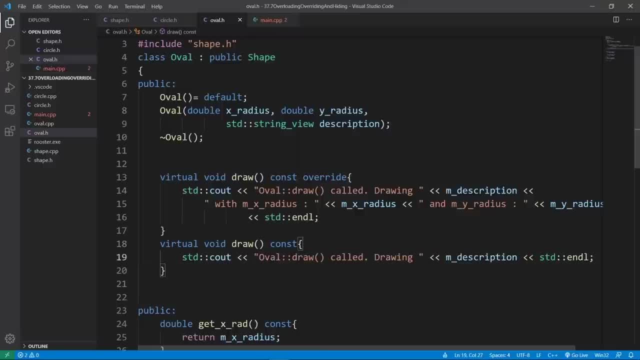 so we can say: overdraw here with the color depth. i don't think we copied the right thing. we can grab this and go in oval and put this in place. this is going to do. we're going to say oval drawing and we can go in circle and also. 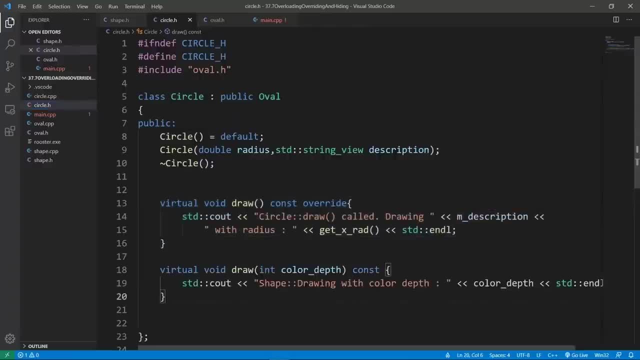 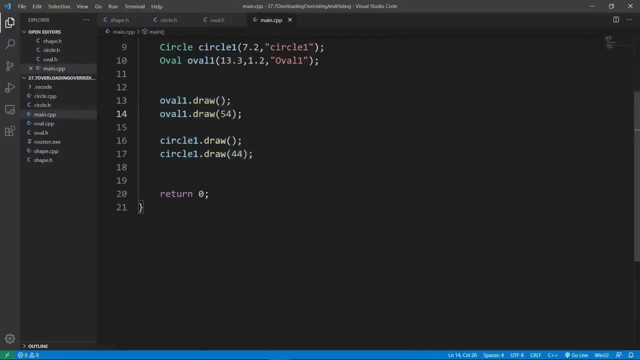 put this in. this is an option and we're going to say circle drawing and now you see that the squiggly lines in main go away because we have overridden all the overloads. okay, if we build and run our program, we're going to see that this is going to work as we expect. 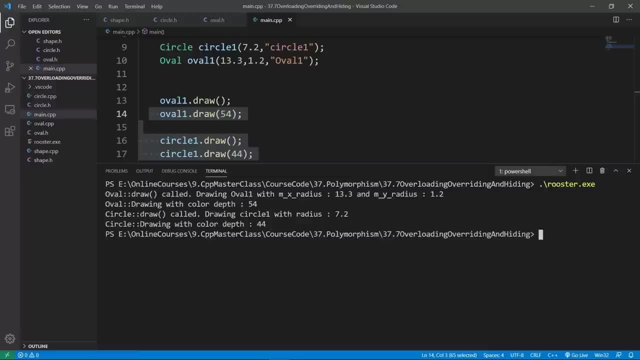 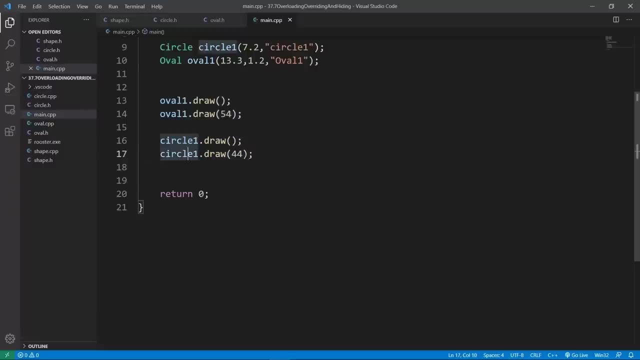 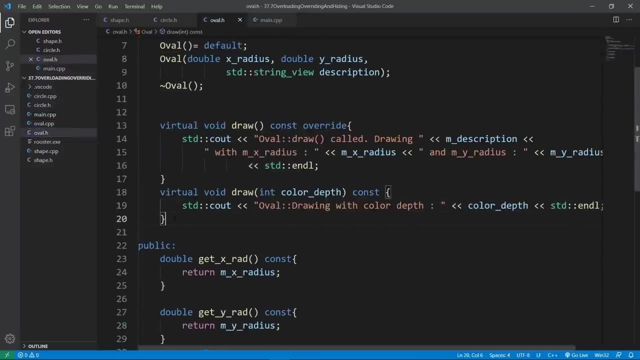 the world is going to be gut and we can clear and run rooster. we're going to see that overdraw called, overdraw called. we are calling our derived overrides and this is really cool. this is what we want here. let's take this back, because we don't want these overridden in our inherited 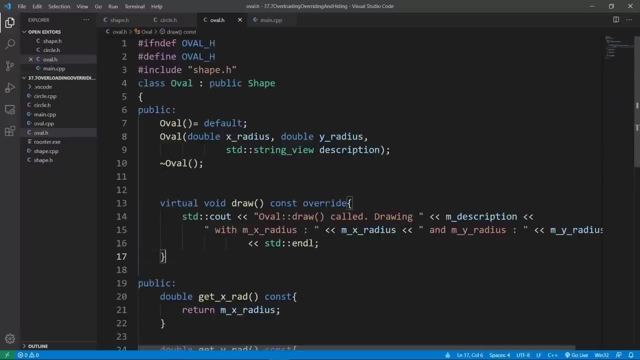 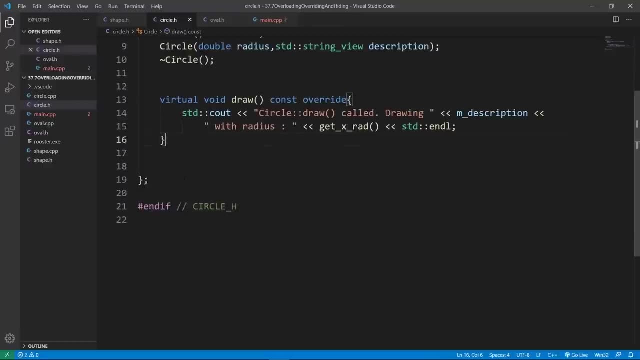 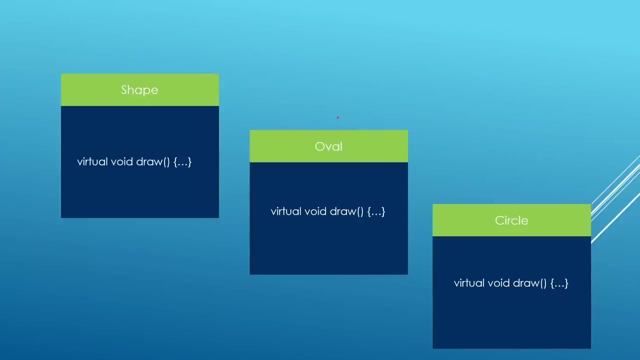 classes. so we're going to take this out in oval and we're going to take this out in circle, and i want you to see that shape polymorphism is not going to work if you overwrite it, overwrite your methods at a downstream level. so what we are going to do, we are going to go at the 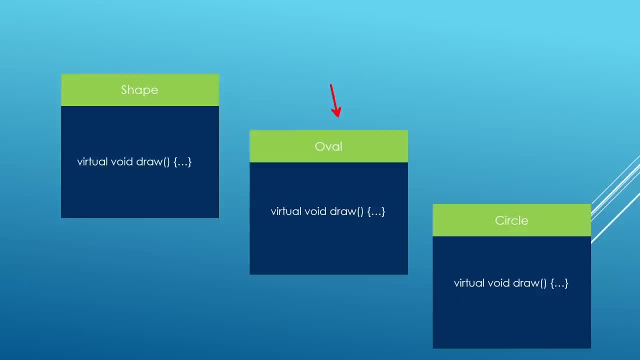 oval level and set up another overload for the draw method here. but this draw method is not going to participate in shape polymorphism because it is really declared at the oval level and any base pointer we have or any shape pointer we have is not going to have any. 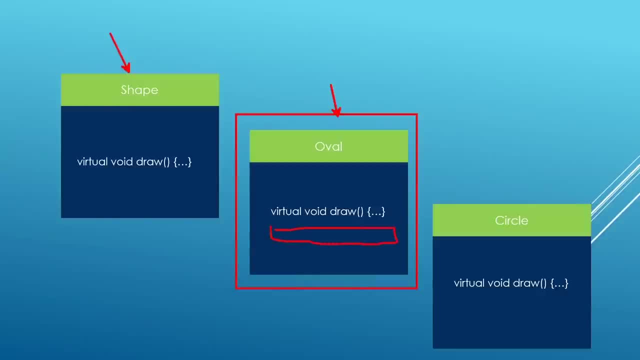 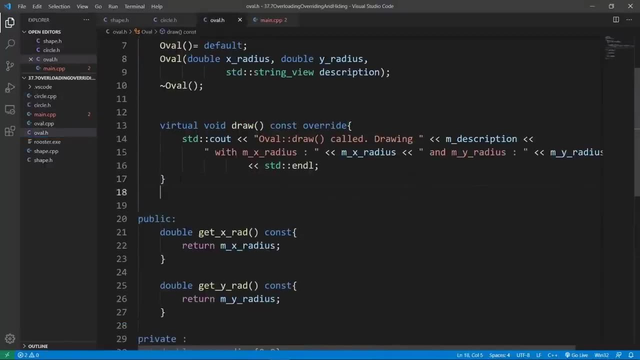 knowledge of this overload that we are about to set up here. this is what i want you to know. okay, so we are going to go in our oval class and set up that overload. we can set that up here. it is going to be taken two parameters. one is going to be the color depth, the other is going 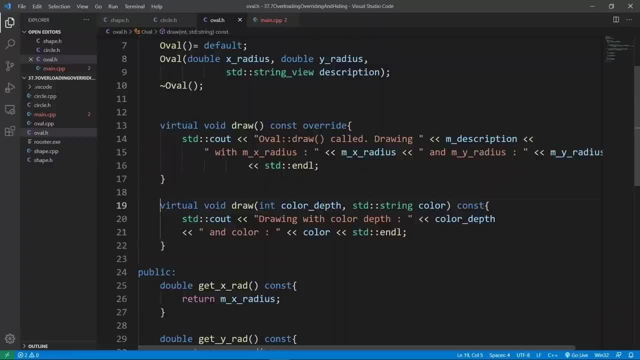 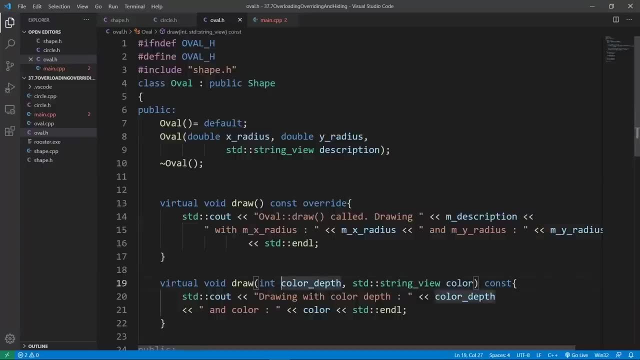 to be the color and we don't want to pass a string by a value like this. we can use std string view and we can include that if we need to, but it looks like visual studio code has got this from something else we have included before, but we can include that explicitly to avoid problems. 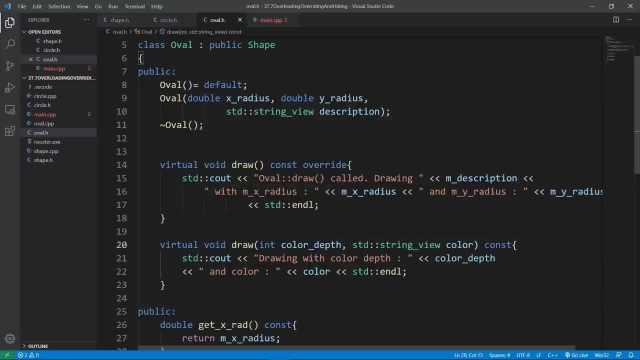 so let's do that. we're going to say string view here and now. we want to see that this method is not going to participate in shape polymorphism, even if it is a virtual functions. the reason, as this is not going to be known by your shape pointers. 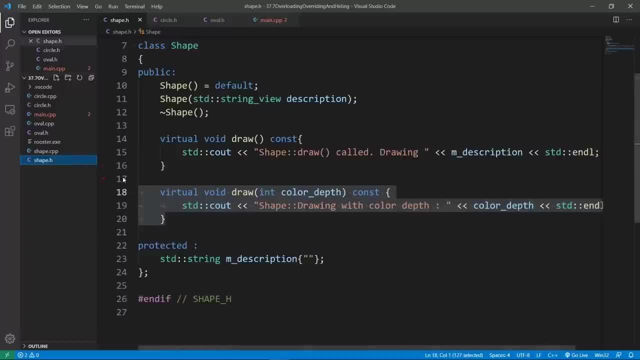 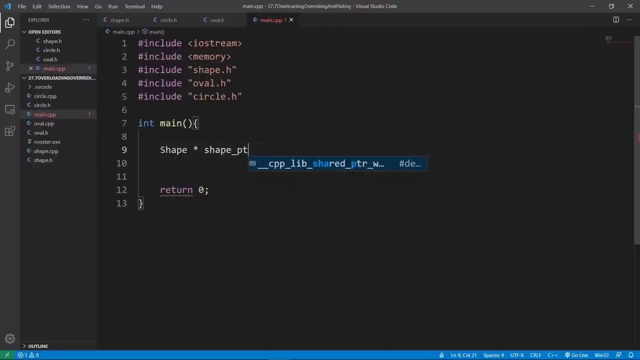 because it is not declared at the shape level. here i really want you to know this: we're going to take out everything we had here and we can set up a shape pointer. we're going to say shape and say shape ptr, and we're going to set up a derived object. here we can say: 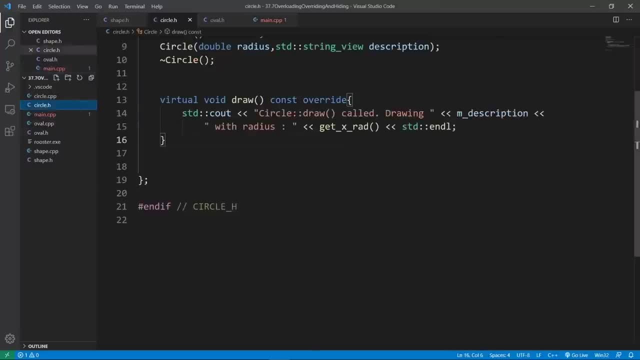 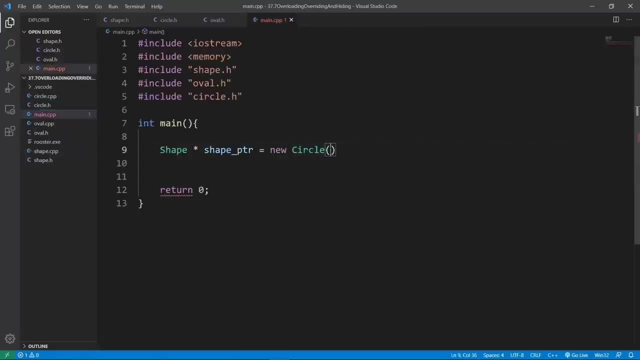 and say circle. and what do we need to build the circle object? we need the radius and the description. so we're going to put that in place here. the radius is going to be something like 10- why not? and the description is going to be circle one. how creative. and we want to see if 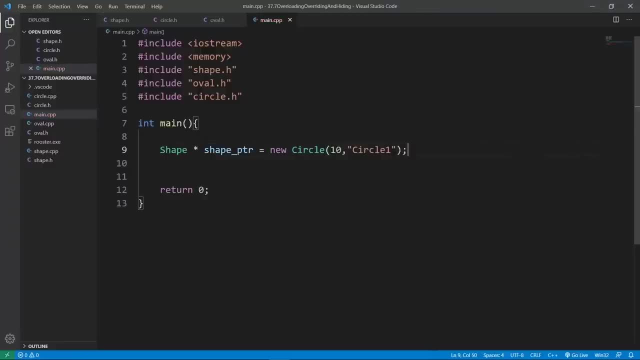 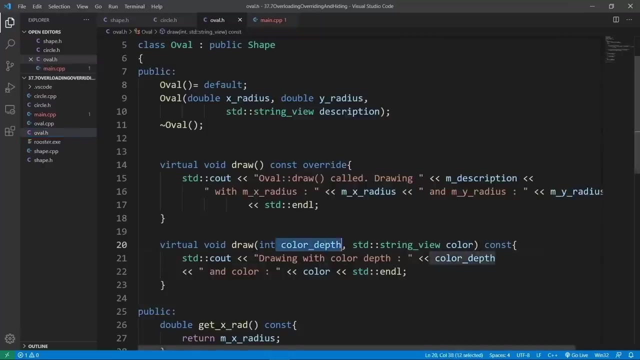 our method is available through polymorphism and it is not going to be available because the method was not declared at the shape level. so if we do shape ptr and say draw, and we have a method which is going to take two parameters, at the oval level we have the color depth and the color. so for 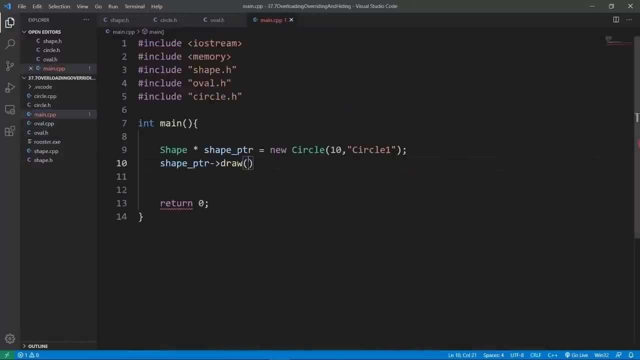 example, if we go in main and say the color depth is 45.2, why not? let's say: this is something that makes sense. or let's use 45, because this is a integer parameter and we're going to pass in a string. let's say red. 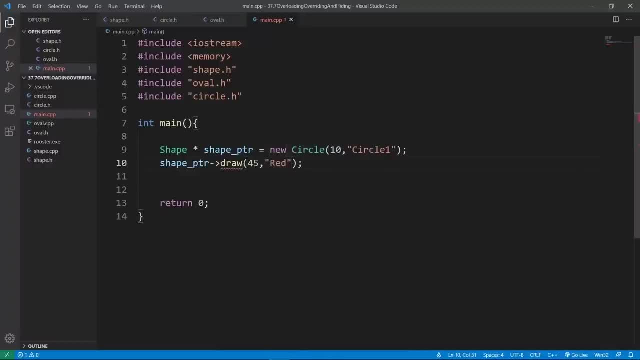 but you're going to see that this is not going to compile because the draw method with two parameters is not known at the shape level. this is the message i want to convey here. so if you want your method to be usable with polymorphism, the method has to show up at the top level. 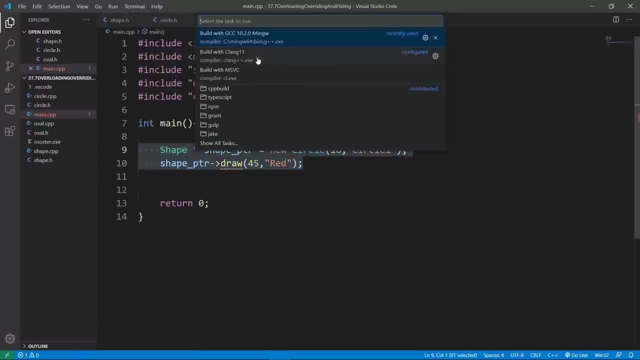 this is what i want you to see here. if we're trying to build this, we're going to get a compiler error and you need to be aware of this. but know that even if this is not working with shape polymorphism, this can work with oval polymorphism, and this is an idea i am going to explore in the next lecture. 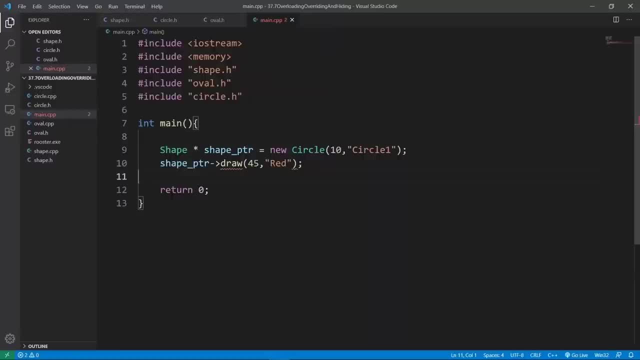 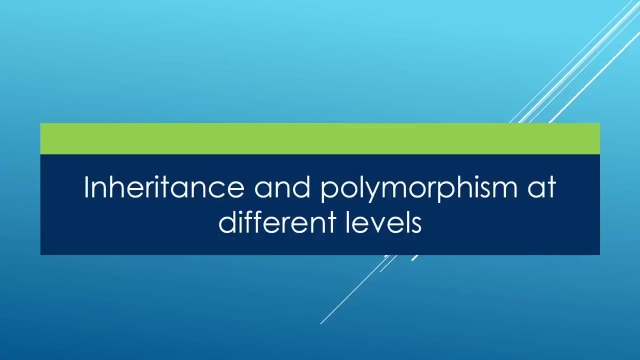 where we learn about the fact that polymorphism can be set up at different levels. so we are going to stop here in this lecture and explore that idea in detail in the next lecture. so go ahead and finish up here and meet me there. in this lecture, we're going to explore the idea that we can do. 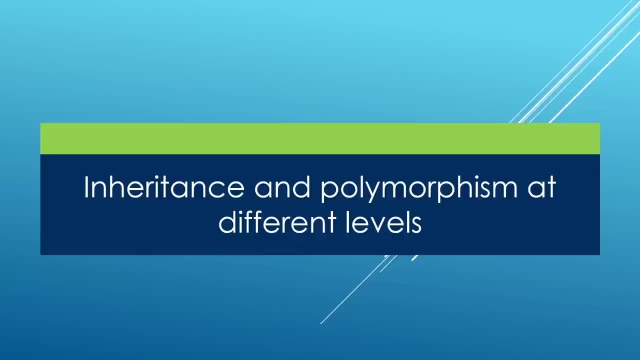 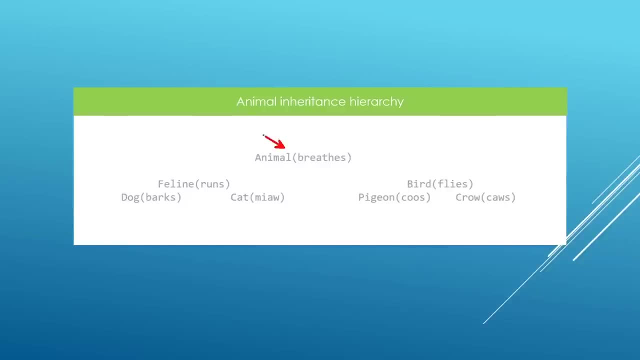 polymorphism at different levels in our inheritance hierarchy. suppose we have a hierarchy like we see here. the top level class is animal and we can derive from animal and create a feline animal. we can derive from feline and create a dog animal. we can derive from feline, create a cat animal. we can also do the other way and create a 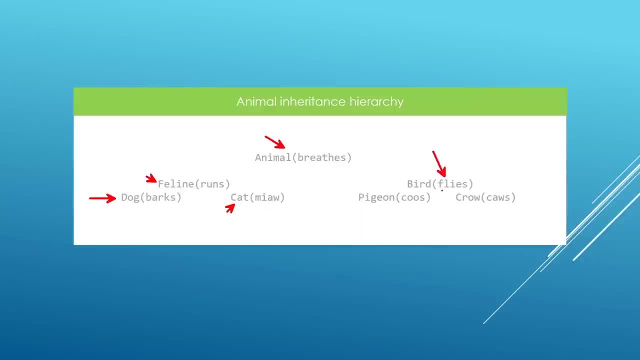 bird, which is also an animal. a bird is going to have its own methods and member variables that make it a bird. we can derive from a bird, create a pigeon, and we can derive from a bird and create a crow, and we can do all these things that these animals do. so the idea you want to expose here is: 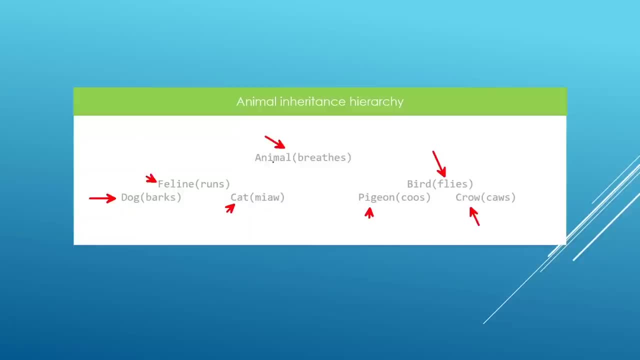 that polymorphism doesn't have to always only work on the top level class. if you have an inheritance hierarchy like this, if you want you can declare a virtual method at the feline level and make sure that method is also available in deriving class and you can set up feline polymorphism if that. 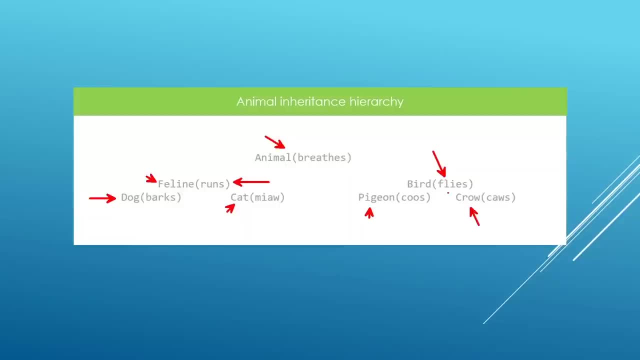 makes sense for your application. following the same idea, you can also set up a virtual method in the bird class and you can have that method overridden in downstream inheriting classes like pigeon and crawl. and you can set up bird polymorphism in your c plus plus program. 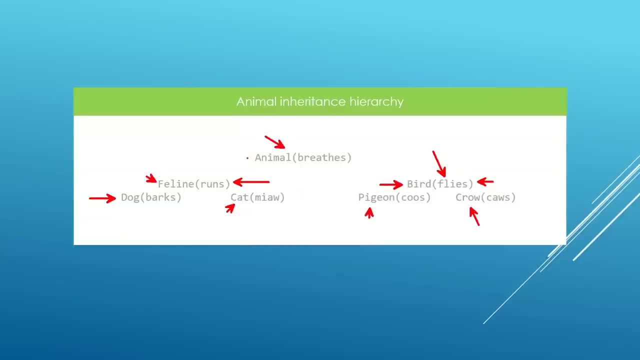 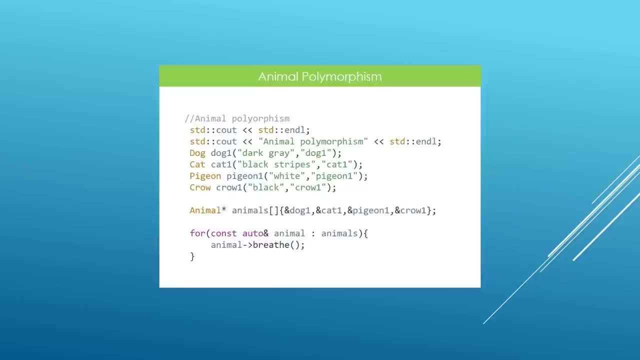 if that makes sense. of course, you can still use animal polymorphism if you want to do that, and that's going to work as well. this is the idea we're going to explore here. okay, so with that inheritance hierarchy in mind, we can create animal polymorphism and animal polymorphism. 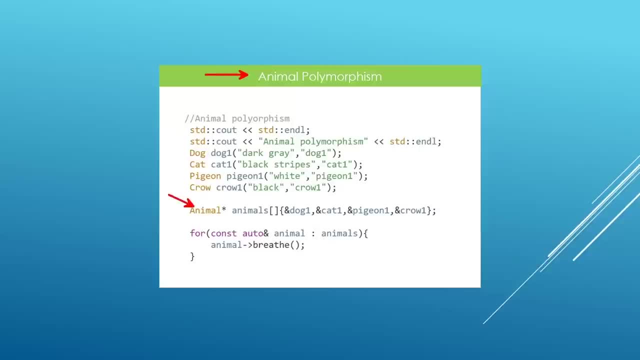 is just going through the animal base pointer and using that to manage derived objects. for example, here we have a dog, we have a cat, we have a pigeon, we have a crow. we can do animal polymorphism and store in any kind of animal we have. here, you see, we are putting in a dog, we are putting 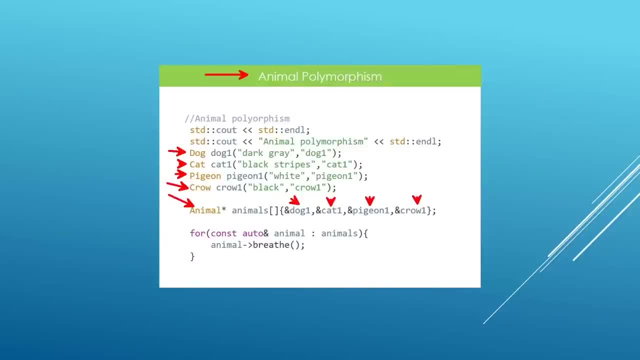 in a cat, we are putting in a pigeon and we are putting in a crow and if we do animal polymorphism and call the breathe method which exists in any kind of animal we have in our program, this is going to call the most specific breathe method on each animal and this is going to work really well. 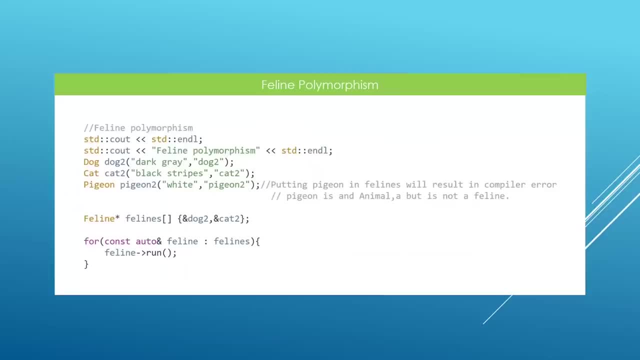 this is going to do animal polymorphism. following the same idea, we can also do feline polymorphism and in this case feline is going to be acting as our base pointer. so again, we have our dog, we have our cat, we have our pigeon. if we do feline polymorphism, we will have to put in all kinds of crazy felines we have. 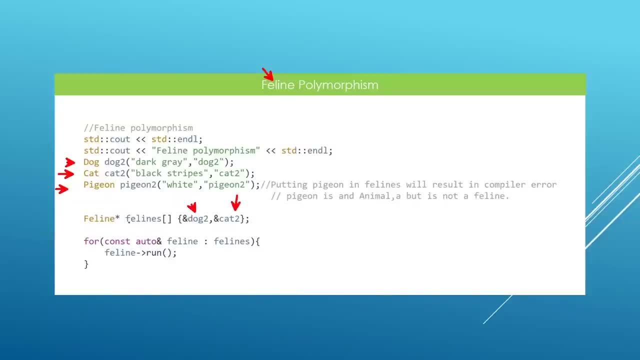 in our program, for example, we can put in dog and cat and this is going to work. if you do feline- a polymorphism like we are doing here- and put in an animal, this is not going to work because the animal top level class is probably not going to override the 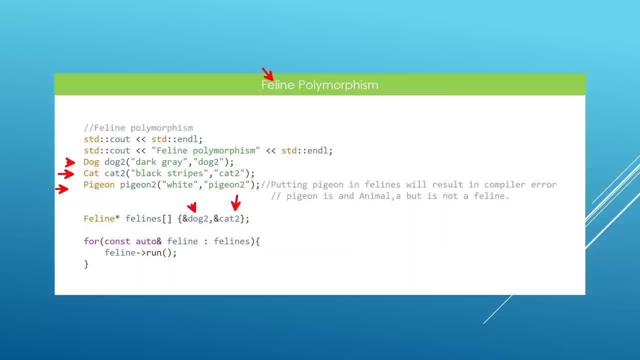 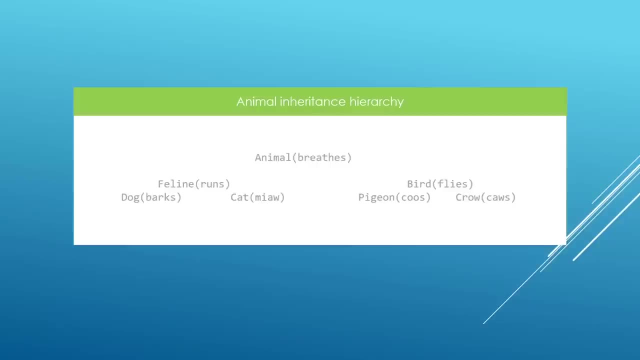 virtual method we are interested in here. for example, here we are calling the run method, and the run method is not set up at the animal level. let's go back and look at our inheritance hierarchy. here you see, this is our animal class. our virtual method is going to be breathe, because any kind of 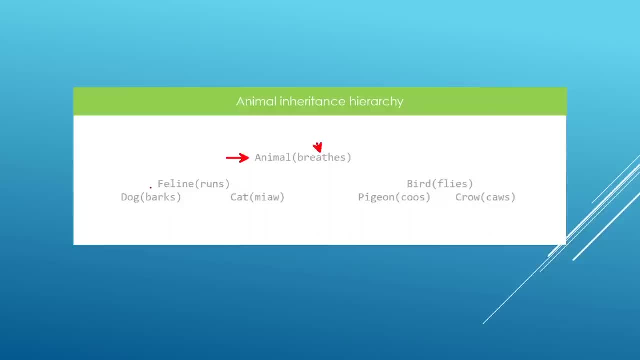 animal we have is going to need to breathe, but the run method is set up at the feline level. so if we try and store an animal in a setup that uses feline polymorphism, the run method is not going to be available and we're going to get a compiler error. 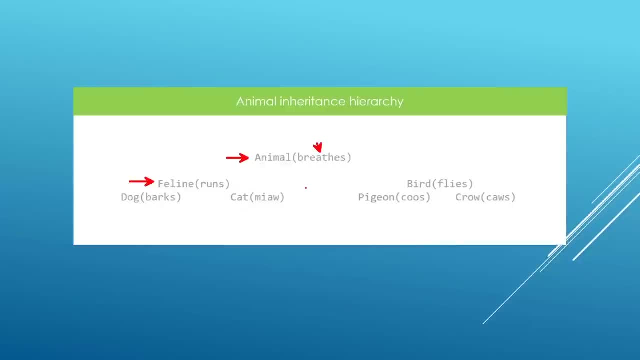 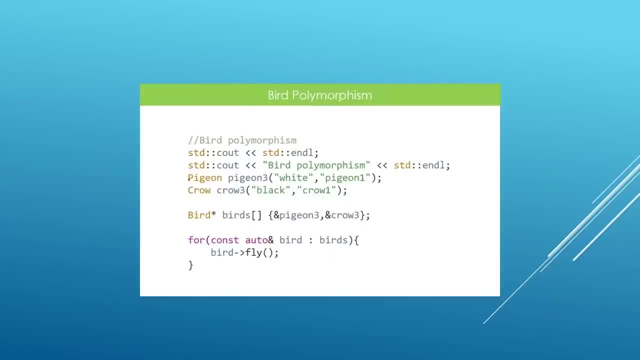 so i want you to notice, but we will also see this in a minute when we hit visual studio code to really play with us. okay, we can also do bird polymorphism. and here you see, we have two objects- one is a pigeon, the other is a crow- and we're going to do bird polymorphism here and what that. 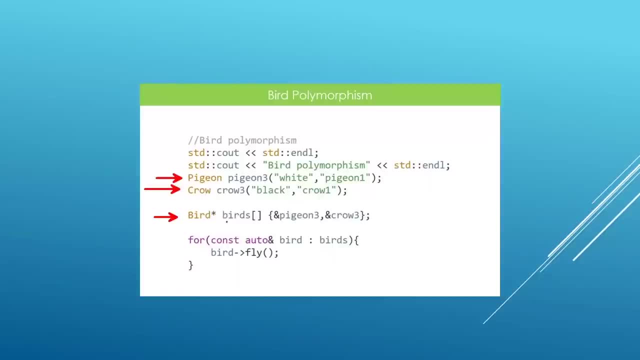 means is that we will use a bird pointer to manage all kinds of crazy birds. in our c plus plus program, for example, we can use that to manage a pigeon, we can use that to manage a crow, and if we look through our birds and call the fly method, the most specific fly method is going to be called. 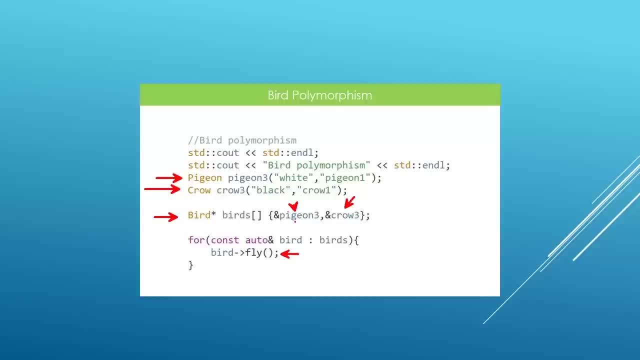 in this case, at the first iteration, we're going to call the fly method on our pigeon object. at the second iteration, we're going to call the fly method on our crowd object here, and this is going to work. now that you know this, we're going to head over to visual studio code. 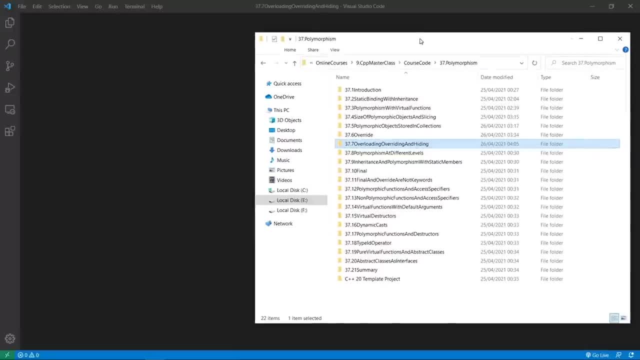 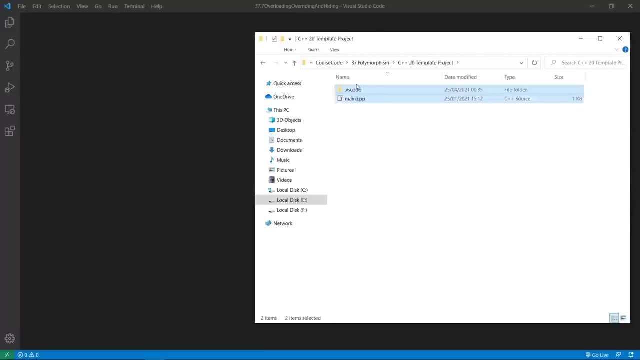 and play with us a little more. here we are in our working folder. the current project is polymorphism at different levels. we're going to grab our template files- let's grab it all. we're going to copy this and put this in our current project and we're going to open this little guy in visual studio code, like we always. 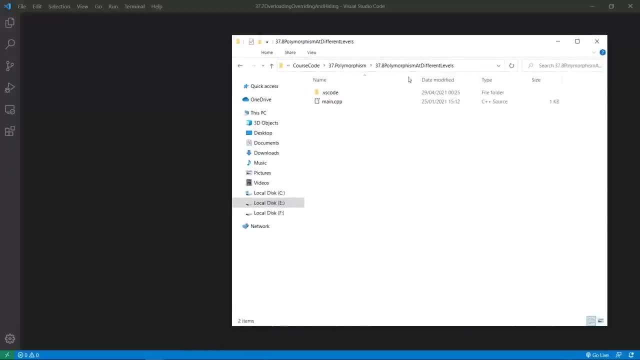 do and before we open this up, i am going to put in the classes i have lying around on my drive and these are going to be the classes making up our inheritance hierarchy. here, to make things go faster, if you want, you can grab these classes from the attached resource section on this lecture. 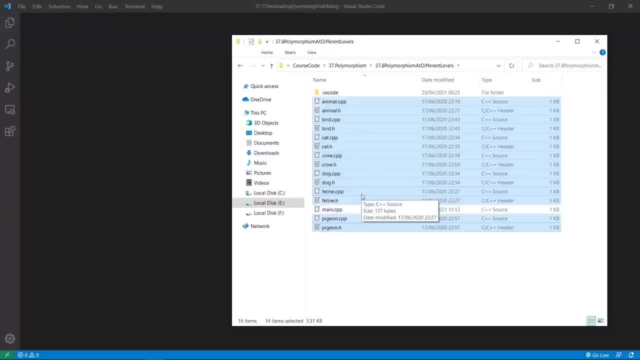 you're going to find all these files. you can download them and put them in your project and use that as a starting point, because you don't really want to be creating all these classes. this is going to just waste your time. the basic idea i want to expose here is doing polymorphism at 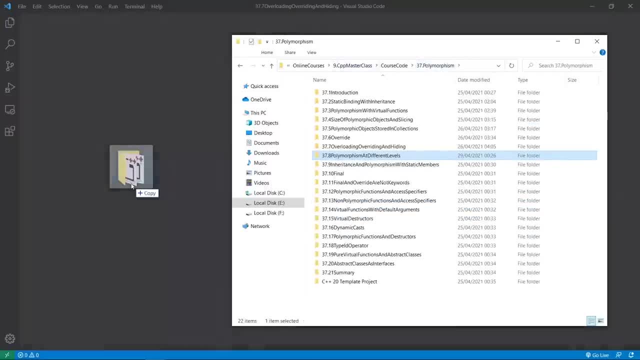 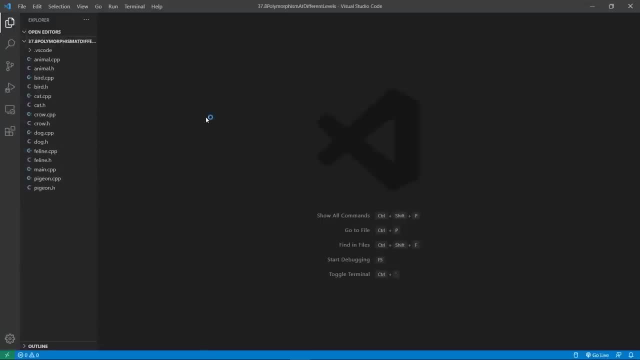 different levels. so we're going to open this up in visual studio code by dragging and dropping here. this is going to give us our good starting point. you see, we have a bunch of classes in here, but all these classes are really trying to set up the inheritance hierarchy. we have here the top class. 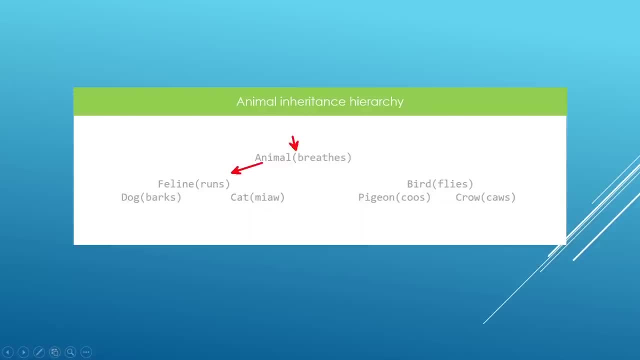 is going to be the animal class. we can derive from animal and create a feline class, and we can derive from animal and also create a bird class. we can derive from feline and create a dog. we can derive from feline and create a cat, and we can also derive from bird create a pigeon. we can also. 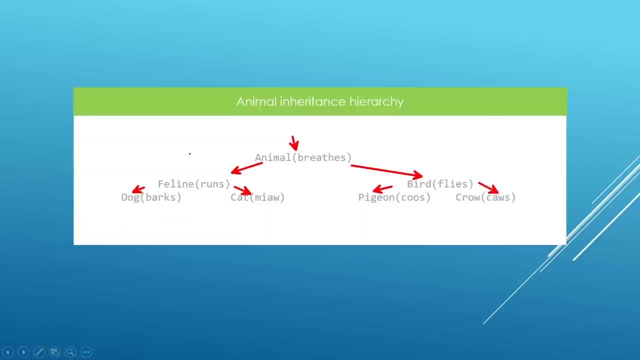 derive from bird and create a crowd class and at each level we're going to have a virtual method that we set up that other deriving classes can call through polymorphism. for example, if we do animal polymorphism, we will get the correct breathe method called, regardless of the actual. 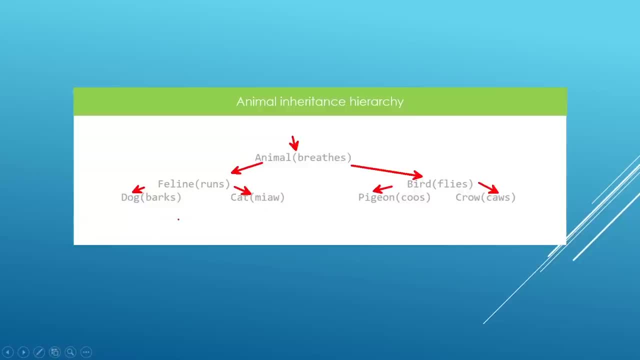 object we are managing with our animal pointer. if we do feline polymorphism, we can manage our objects through feline pointers, but we will get the correct run method called, regardless of which kind of object we are calling this method on. so if we call the run method on a base pointer managing 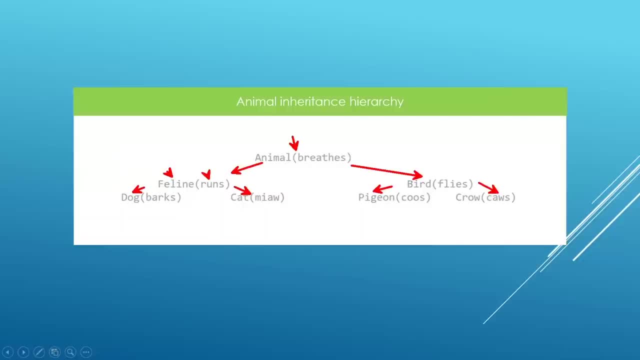 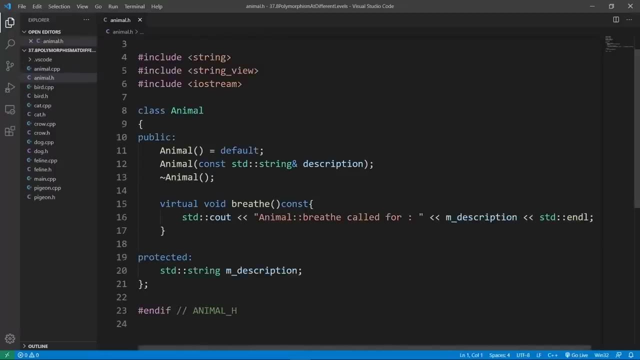 a dog object, we will get the run method called on the dog object. this is what we mean here. okay, so we have our classes here. let's take a closer look at our animal pointer. so we are going to call this animal class, it is our top level class and it is going to have a virtual method which is called 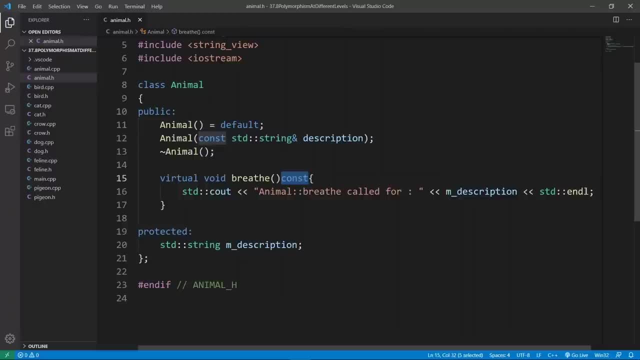 breathe. it is cost because it is not modifying our class here. notice that we don't have a virtual destructor, because i wanted to keep this simple. but in your practical object you should make your destructors virtual if you happen to have a virtual function in your class here. so, for example, we can 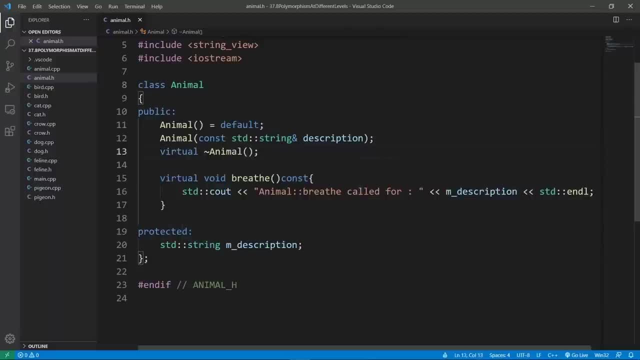 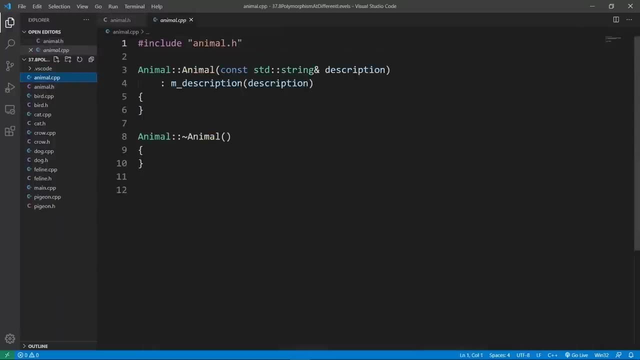 even do that. let's make this virtual. this is not going to cost us anything and this is going to be our top class. we can now look at the implementation file. it is not going to do anything special. it is just going to forward whatever parameter we pass and use that to initialize our member variable. 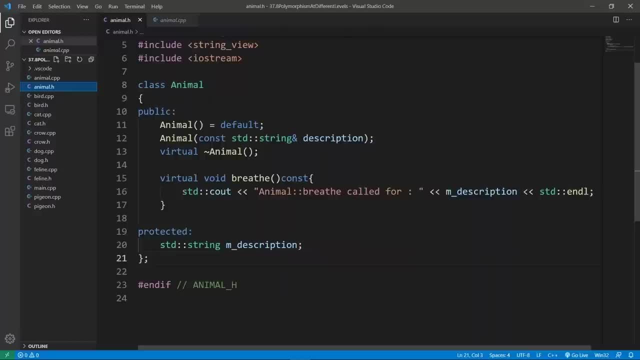 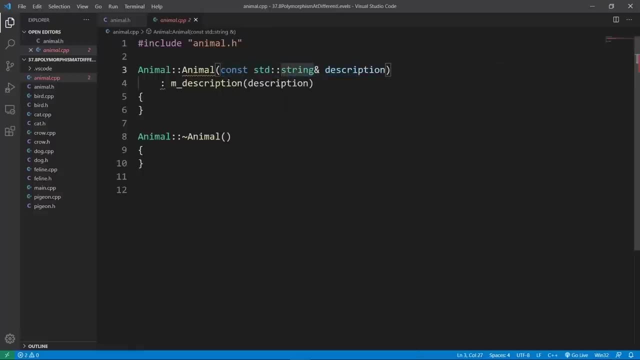 i think we can also go in and change our parameter to a string view. so we can do that std string view. let's go in the cpp file and also change that pretty quick. we're going to say std string view here and this is our animal class. we're going to go in our feline class because 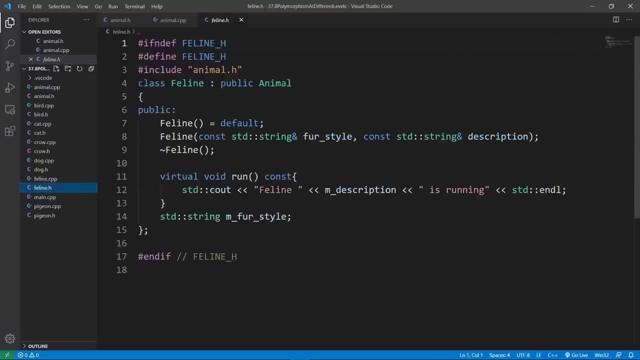 that's the deriving class. feline is going to be inheriting from animal publicly, just as we see here. we're not going to really do anything special. we're going to set up a member variable called first style and we're going to forward the data from our constructor and use that to initialize. 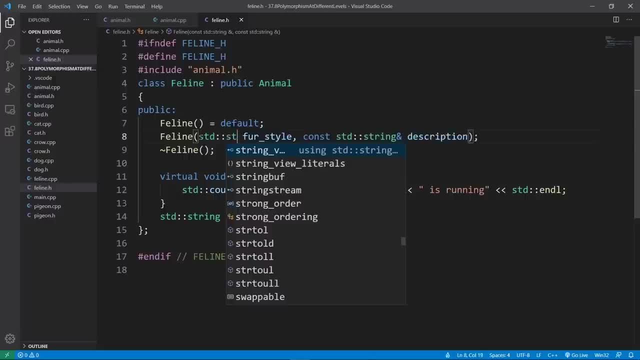 stuff in our class. here our parameters are also going to be passed as std string view types, so let's do that here, and this is in place. we also have a virtual method which is called run, and inside we are just printing which kind of object we have, and 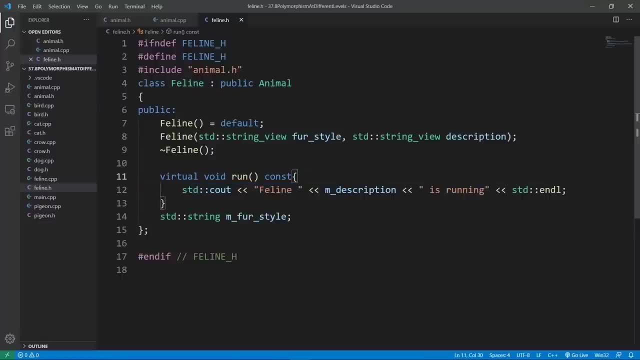 giving a hint on the method that is being called here. this is what we just do here, and we don't intend to create feline objects directly. that's why we're not setting up any overrides of the top. that's why we are not setting up any direct 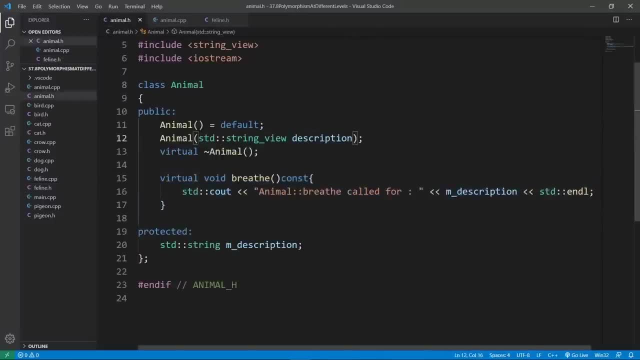 specific overrides for these methods. but we will do that in downstream classes, for example dog and cat, because that's going to make sense there. let's go in the cpp file for feline and also change things a little bit. we're going to use std string view parameters. let's do that for the. 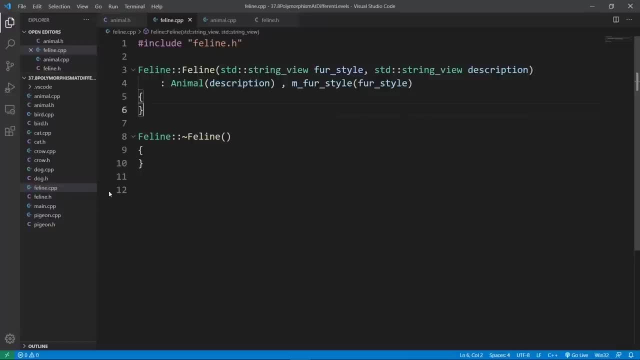 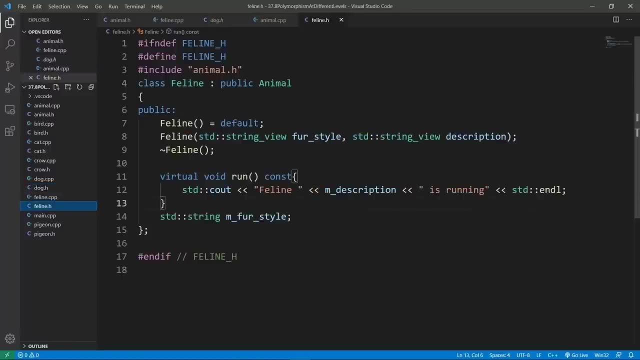 second parameter as well, and this is our feline class. so we can go in and look at our dog class. let's see if we can find it, and i don't think we made our destructor in feline virtual, so let's do and look at our dog class pretty quick. here we have our dog. it's going to have. 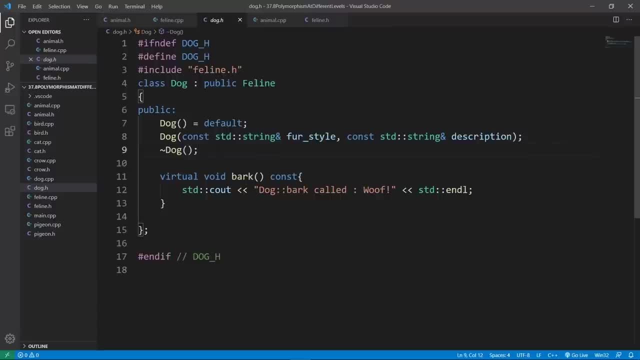 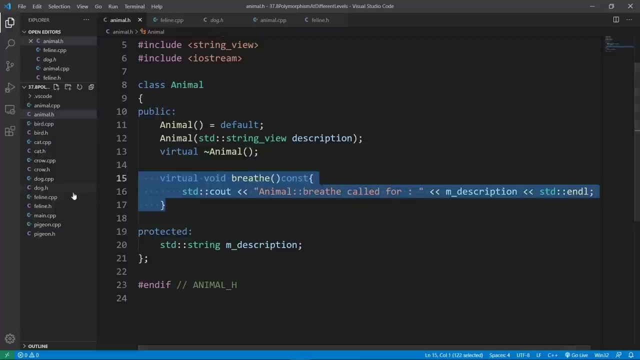 no member variable at all and it will just forward this data to up stream classes. but we can override our breathe method. we get from the animal class. we can do that and we are going to say we can grab this entire thing and we're going to go in dog. we can do that if we want. 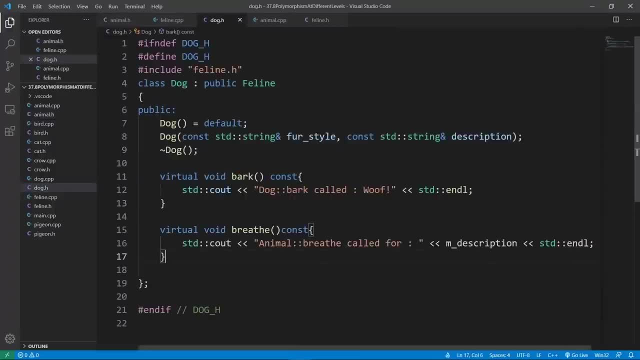 we're going to put this method down below here and we're going to say, breathe. we're going to say that is overriding what we have on top and we're going to say, dog, breathe cold. this is going to do, and we also need to change our parameters to hdd string view. let's do that. this is going to make. 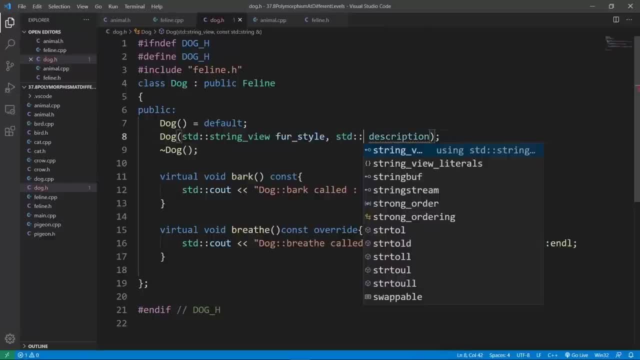 things work better because we will avoid unnecessary copies and we will be able to pass string literals as parameters to this constructor here. this is what we want to achieve. with us, we can hit the cpp file for our dog class and we're going to change the parameters. 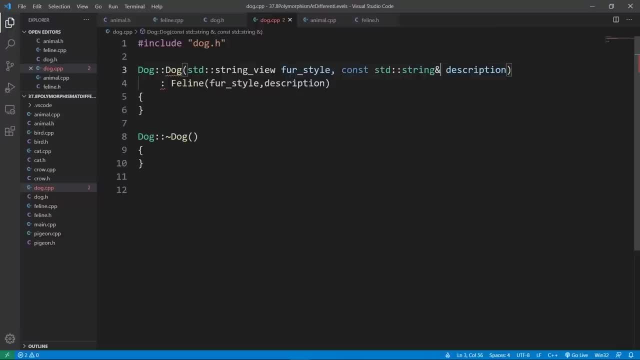 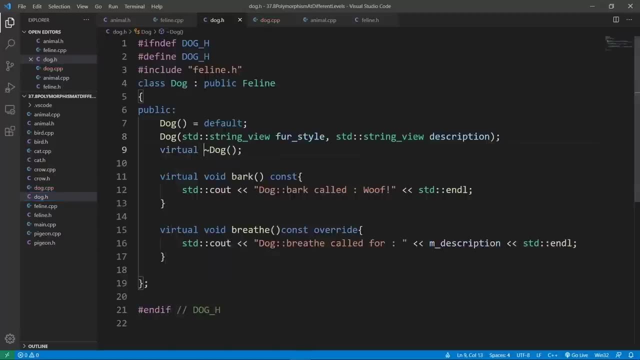 again std string view, and we're going to say std string view as well here, and we're going to go to the header file again and make sure we have a virtual destructor here, because this is good practice. if you are using virtual functions, like we are doing here, we can grab our breathe method. 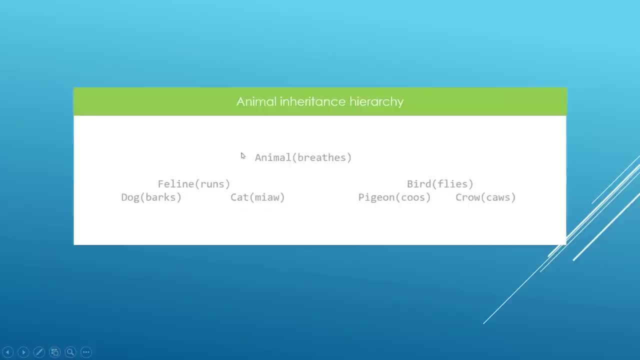 and hop over to our cat class again. remember the inheritance hierarchy we are going after is what we have here, so if you are confused, please come back and look at this. you're going to really understand what we are doing here. we're going to go to the dog class and make sure it is. 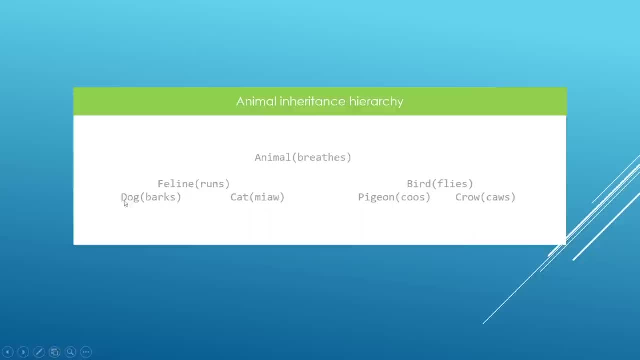 working as we want. so we just did the dog class and we just made sure it works like we want. now we're going to hop over to cat and make sure it is. now we're going to hop over to the cat class and make sure it is overriding the breathe method to make sure the correct method is called. okay. so 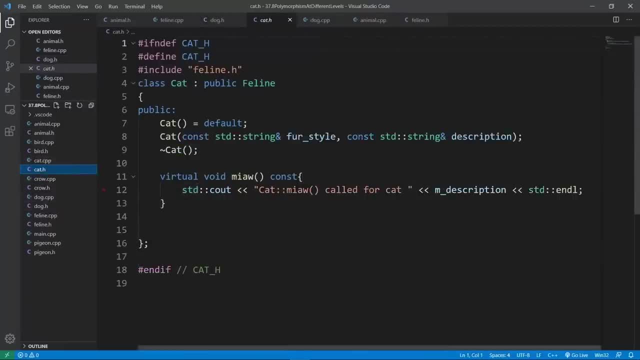 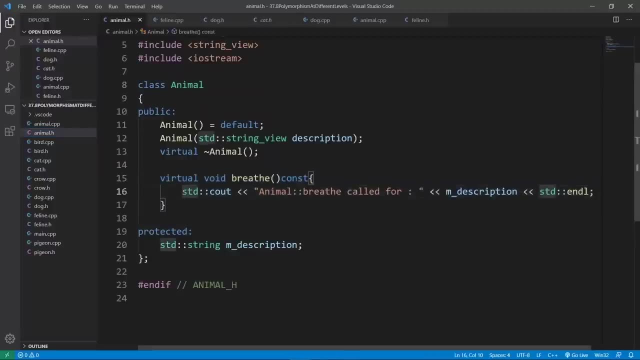 let's do that. we're going to hop over to our cat class. it is going to have its own meow method, but it can also override the breathe method we get from the animal class. so let's do that. we can grab this and we can go to our cat class. let's. 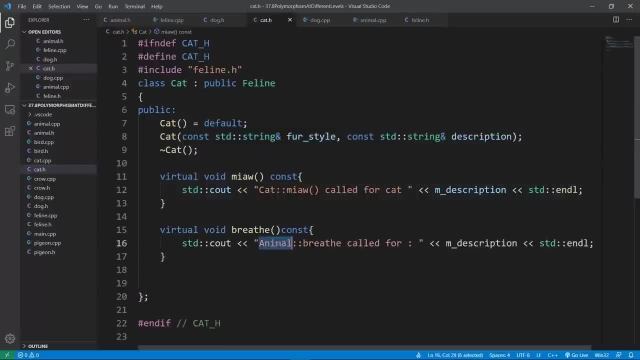 do that. we're going to put in our virtual method and we're going to say: cat breathe, and this is really all we also need to set up our parameters correctly using std string view. let's do this std string view and this is really all we need to do here. we can also make our destructor virtual, because this is good. 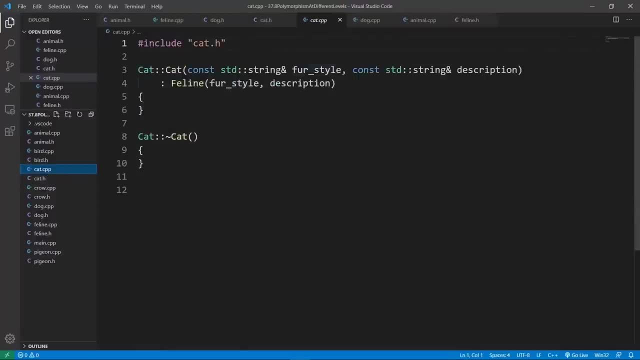 practice, we hop over in the cpp file and change our parameters to be of type std string view. let's do this and this is done. we can really work with this inheritance hierarchy here. we're going to also go pretty fast and work on the other side of our inheritance hierarchy. we're going to work on. 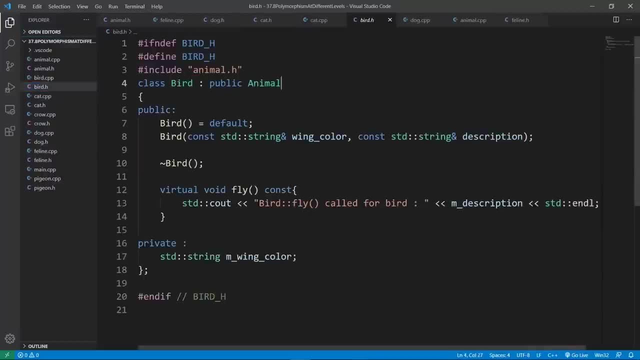 birds. let's look at the bird class. it is going to inherit from animal class and this is going to be multiple breed lines. but we're not going to do anything special really. but we just want to change the type of our parameters to std string view and we're going. 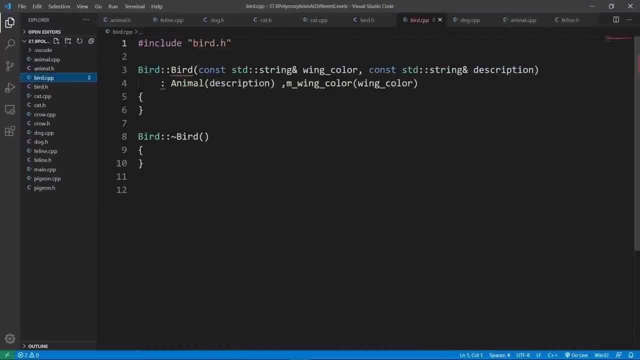 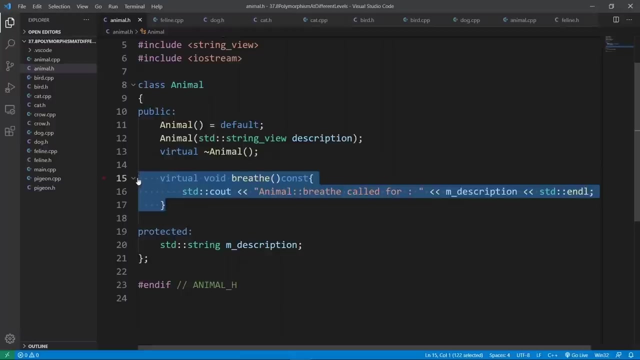 to do that on the second parameter and we are going to hop over in the cpp file and change these things here. let's do that. we're going to say std string view and do the same thing here- std string view- and the bird is done. we can grab our breathe method, for example. let's go back. 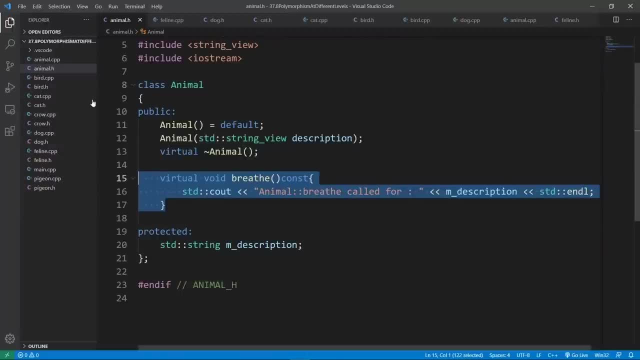 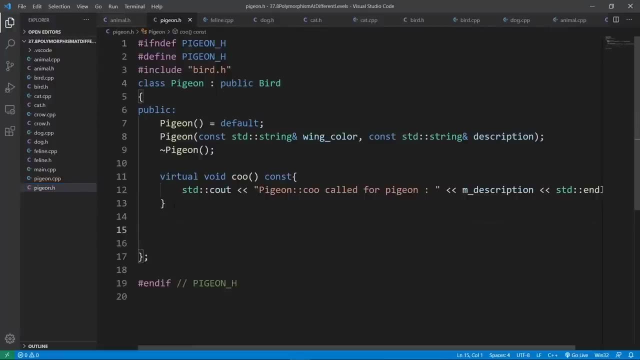 to the top and grab that from our animal class, one kind of bird we have in our program. we can look at pigeon, for example, the last class. here we're going to override the breathe method and we're going to say pigeon breathe, and we are going to change the type of our parameters here to std string view and we're going to do the same. 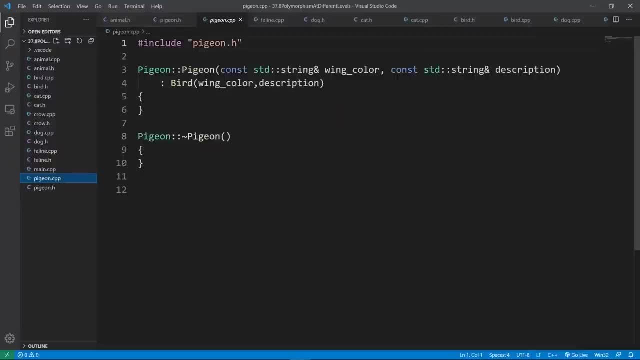 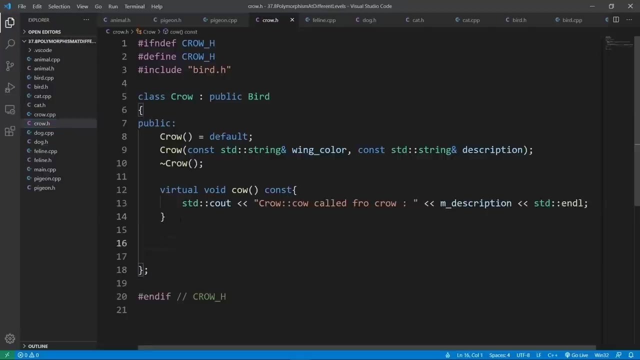 here and let's hop over to the cpp file and change the type of our parameter. let's do that for the second parameter. here this is done. let's look at the second kind of bird we have. i think we have the crow class. we also want to override the breathe method. we're going to say crow breathe. 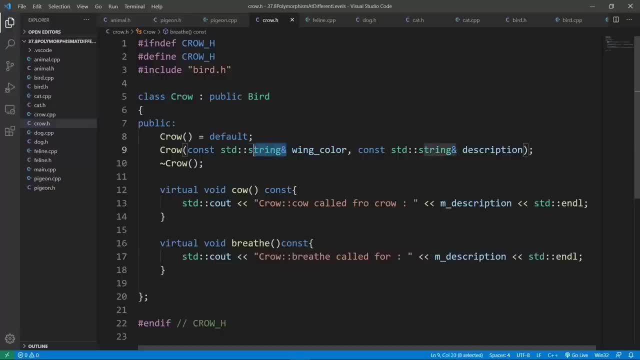 and we can go up and change our parameter to be of type std string view, and we're going to do that here again. if you are not interested in these changes, you can just grab the code and you're going to have all these classes ready for use. 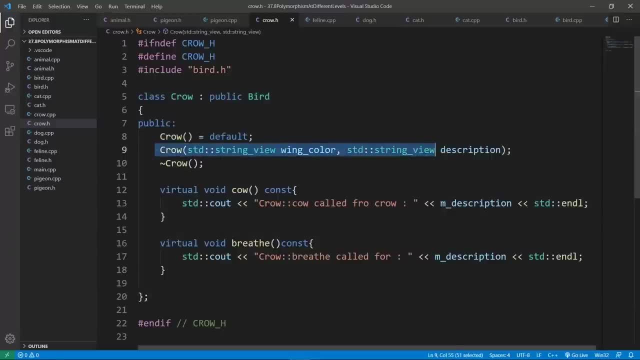 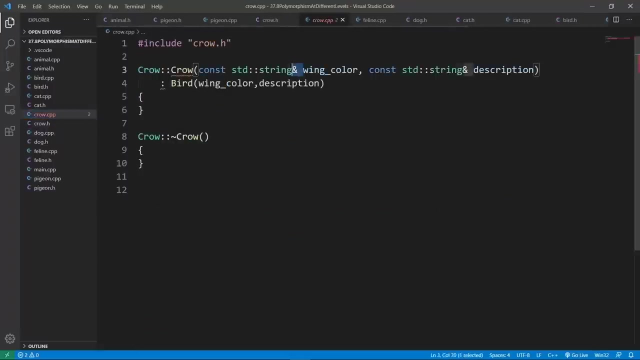 i just want to to correct this little problem i had in my classes on my drive, because this is not good to design in modern c++. we want to do things proper because we are really learning about modern c++ here. let's hop over to the cpp file and finish this up. we're going to change the type to std string view. 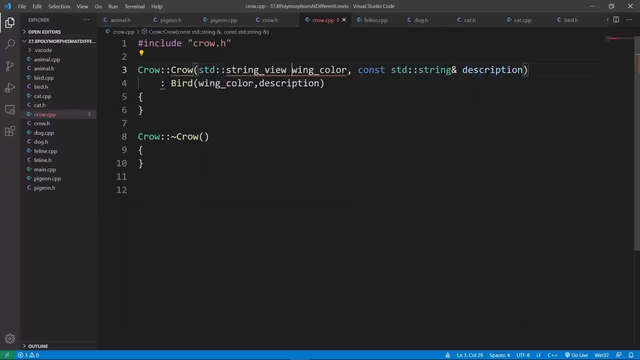 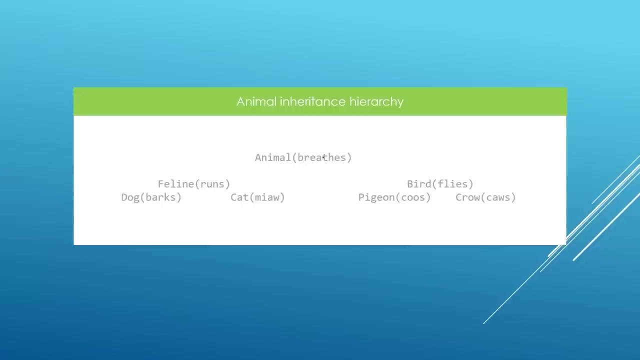 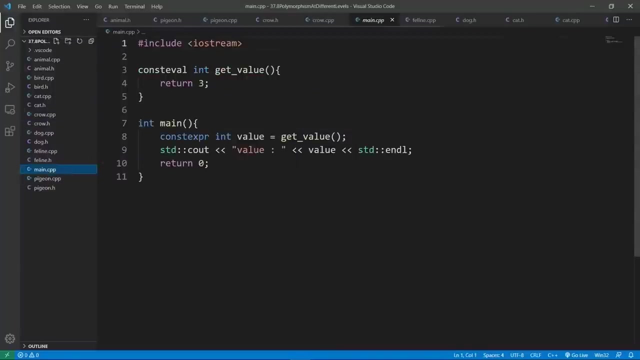 and let's do view correctly and we're going to say std string view on the second parameter, and this is done. now we have our inheritance hierarchy and we're going to start by looking at animal polymorphism. again, we just set up this inheritance hierarchy. now we are going to try and do animal polymorphism okay. so now we're going to hop over to the main cpp. 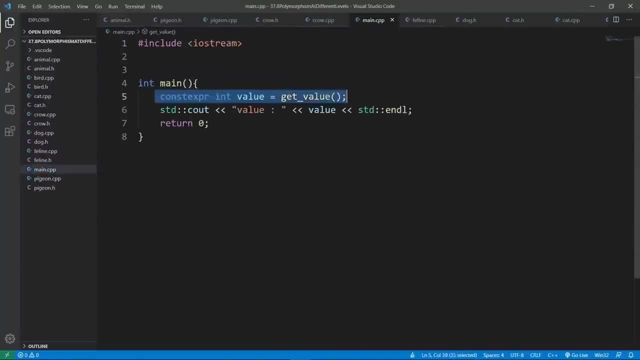 file and we are going to clean it up a little bit, remove whatever it is we don't need. we are going to put in our includes. we're going to include all of the things in our file here: animal, feline, dog, cat, bird, pigeon and crow. we're going to include all this. 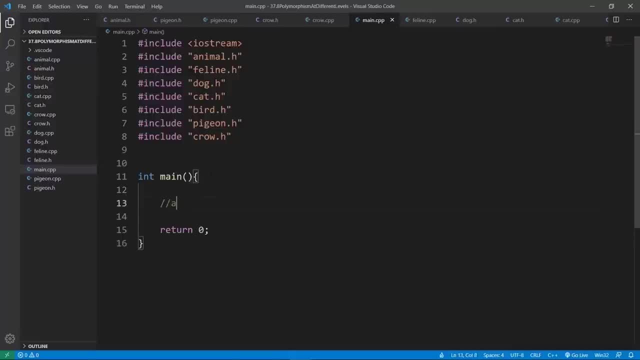 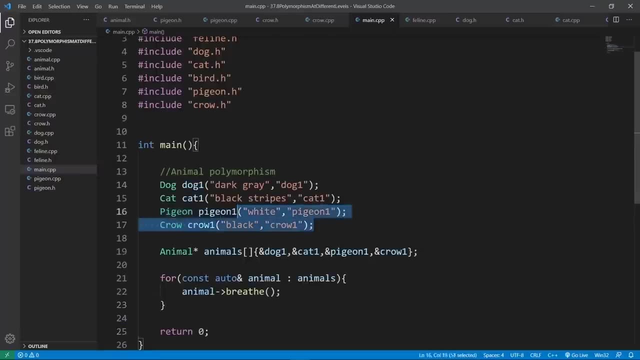 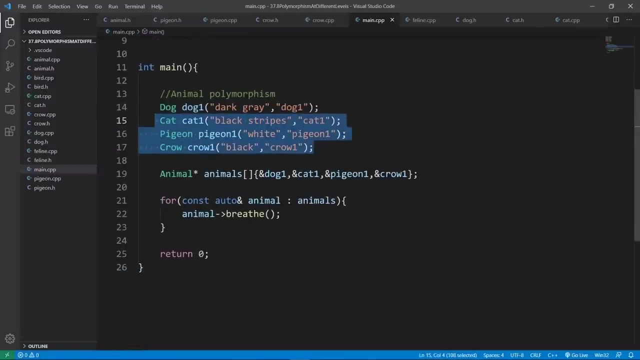 and we just want to play with animal polymorphism here. we are going to set up a bunch of objects and we're going to put in dog, cat, pigeon and crow- all kinds of crazy animals we can create in our c++ program- and we're going to put them in an array that is storing animal pointer and this. 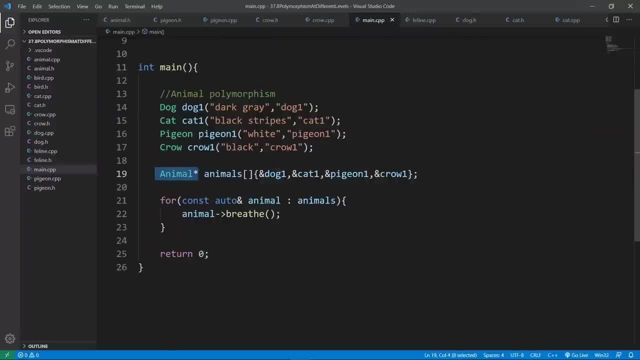 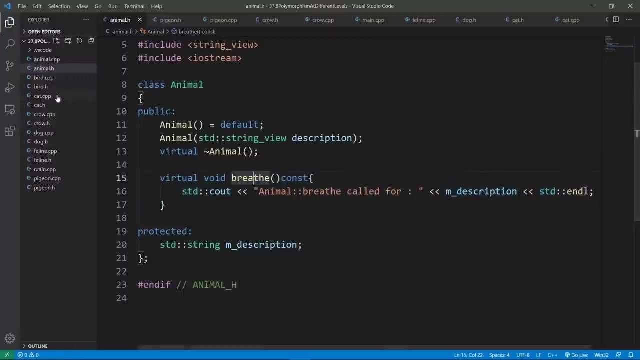 animal pointer is going to enable polymorphism for our objects that we have in here. remember, animal sets up a virtual method called joe- if we go back we're going to find that- and we made sure to override this method in all kinds of crazy animals we can create, for example in our cat. we. 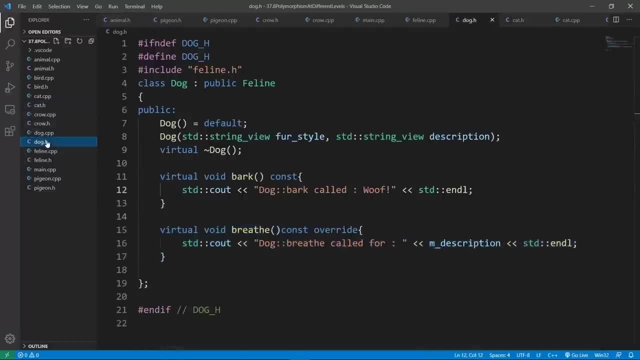 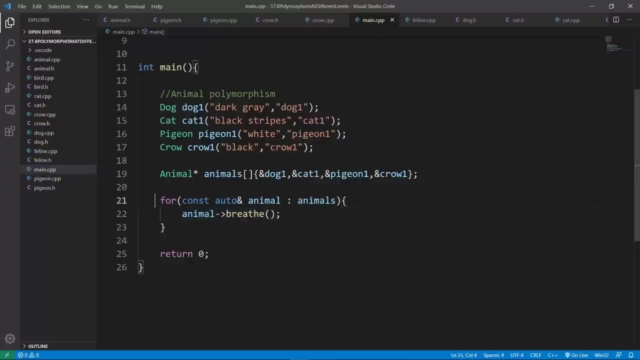 have a breathe method overridden in our dog class. we have the breathe method overridden and what we want to achieve in our main cpp file- let's go there, if i can find it- we want to achieve a setup so that if we call the breathe method, we're going to call the 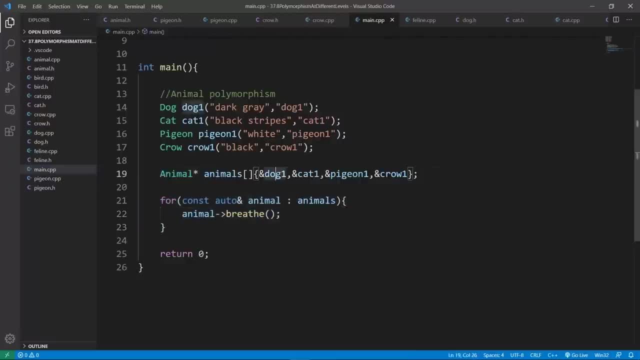 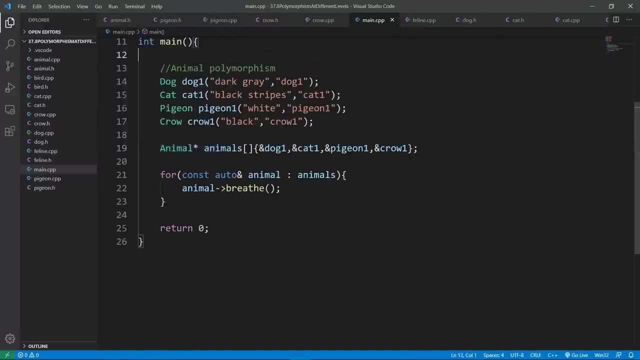 most specific breathe method on our animal pointer here, even if we are calling that method on a base pointer. this is what we want to achieve. this is going to be animal polymorphism, because the base pointer is of animal type. this is what we mean here. let's try and build this program so if we 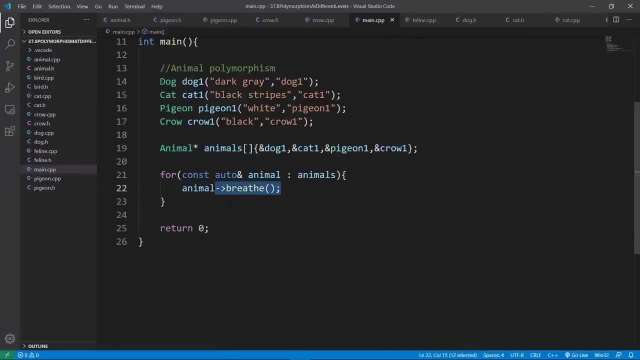 loop and call the breathe method. the correct breathe method is going to be called and what we expect for the first object, which is a dog object, we're going to get the dog breathe method called. for the second iteration, the cat breathe method is going to be called for the third. for the third iteration, the pigeon. 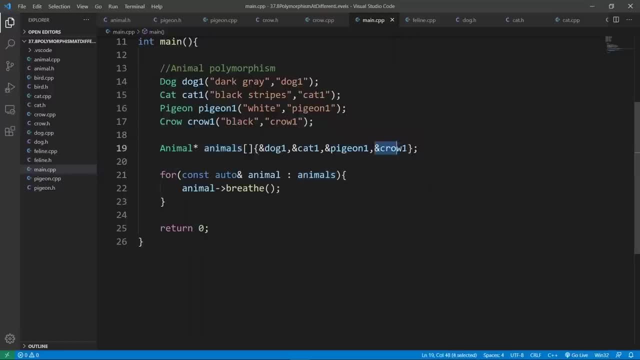 breathe method is going to be called for the last iteration, the crow breathe method, is going to be called. this is what we expect to see if we run this program here. so let's do this. we're going to pass this through gcc, our favorite compiler. we can use any compiler we want, but gcc is going to. 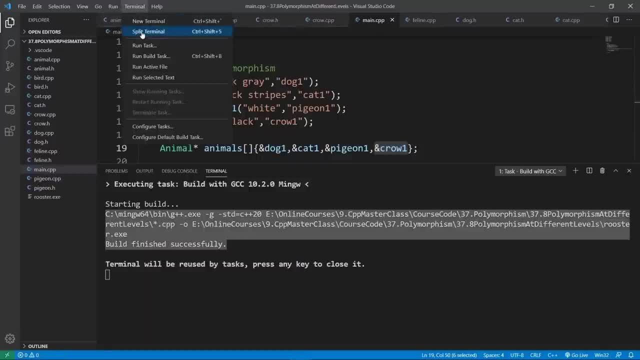 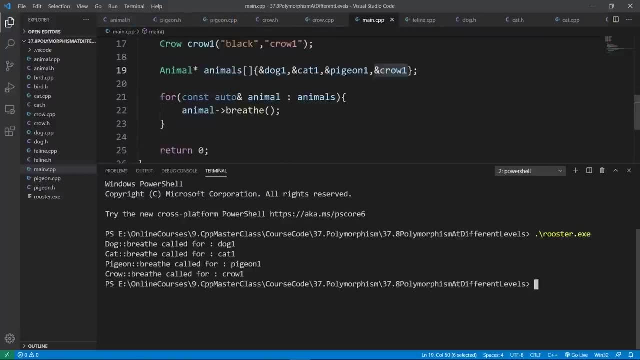 do in this case? okay, the build is good, we can bring up a powershell window to play with the build and we're going to run rooster our program and if we run this, you're going to see that in our loop. the first iteration is going to call dog breathe, because the first object is a dog. 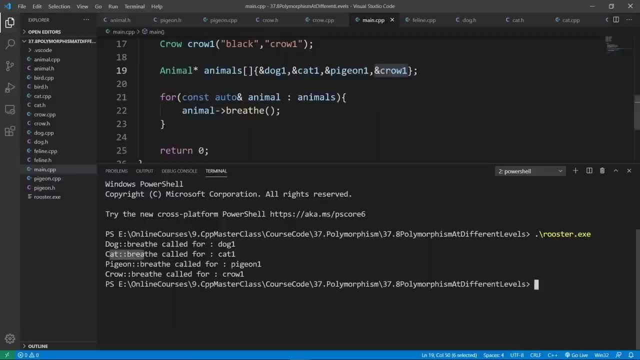 the second iteration is going to call cat breathe, because the second object is a cat. the third iteration is going to call pigeon breathe, because the third object is a pigeon, and the last iteration is going to call crow breathe, because the last object is a crow. and notice that we are calling the breathe method through a base. 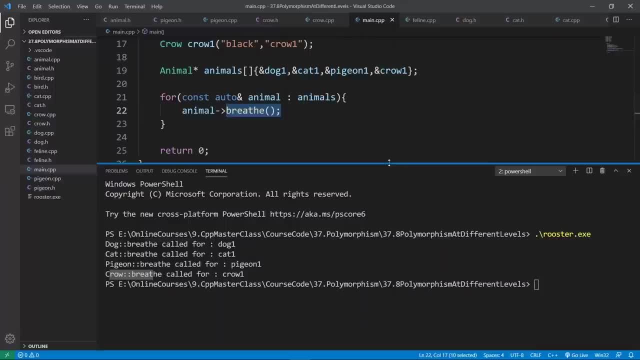 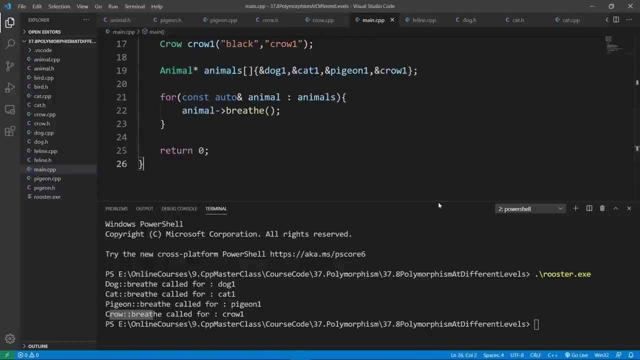 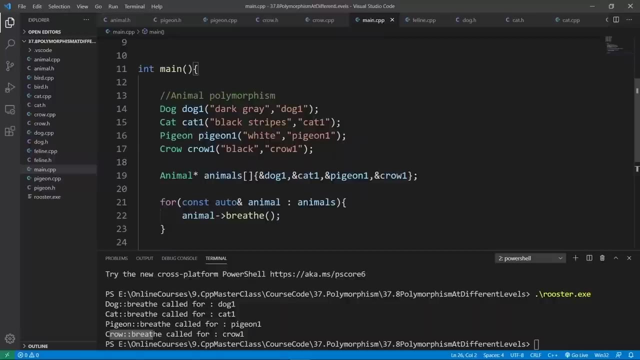 animal pointer, and this is what polymorphism is all about, and what we are doing here is animal polymorphism. but this is not what we are really after in this lecture. we want to see that we can also do feline and bird polymorphism in our inheritance hierarchy, so we're going to put 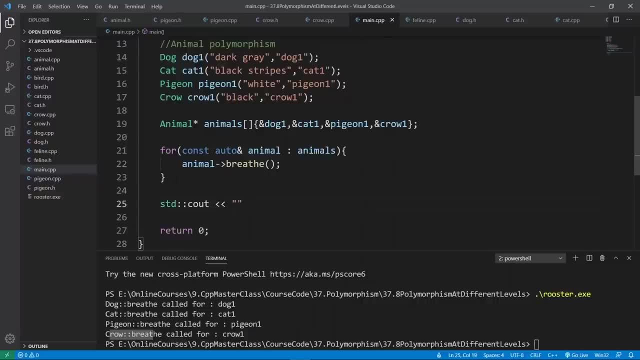 in a separator. let's do stdc out and put in a bunch of dashes here or hyphens, some people call them- like that doesn't really matter. and we're going to do this animal pointer and this is what we're going to play with feline polymorphism. let's do this. we are going to go down and put 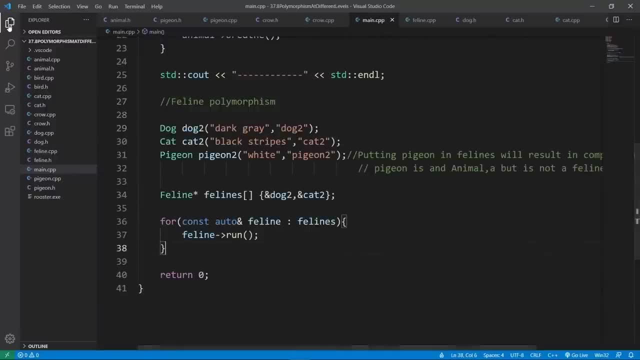 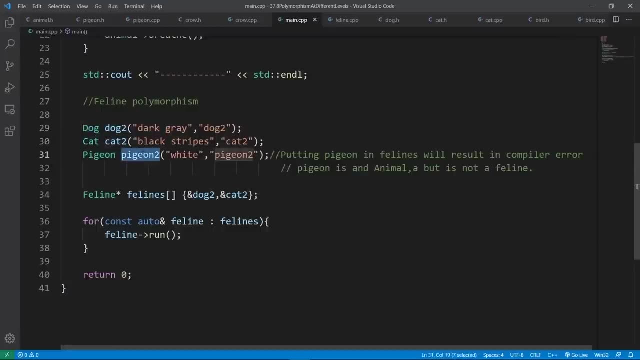 in a simple piece of code that we're going to be using to play with things here and we're going to set up a bunch of objects. we have a dog, we have a cat, we have a pigeon and we are going to use a feline pointer to manage feline derived objects. for example, we're going to use this pointer to 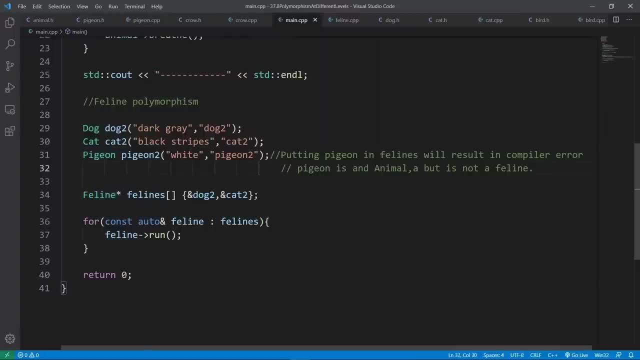 manage a dog and a cat, but one thing i want you to see is that if you put in a pigeon, for example, this is not going to be a dog and a cat, but it's going to be a pigeon and it's going to be a dog. 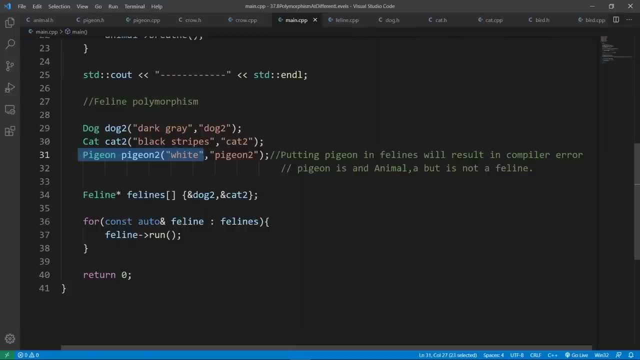 because a pigeon is not a feline, so the compiler is going to give you a compiler error. let's try and do that. we're going to try and put in pigeon here, pigeon 2- you can select this, and if we do that, you're going to see that we get a squiggly line. this is a sign that this is going to go wrong. 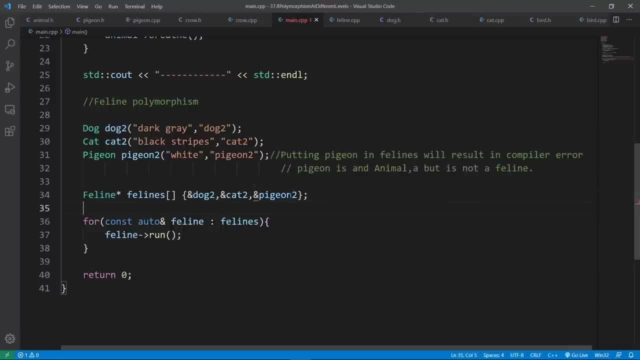 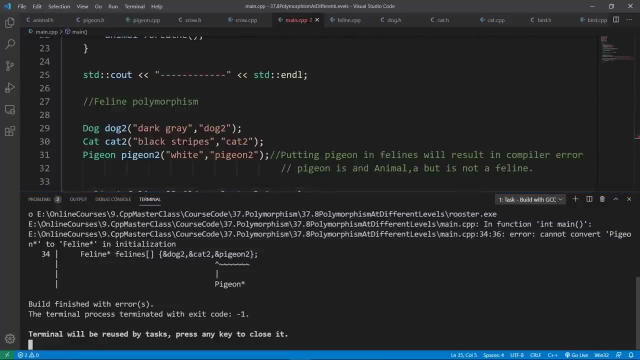 because we are storing in felines and the pigeon is really not a feline, even by our inheritance hierarchy. so the compiler is going to give us a compiler error. let's try and build to show you the compiler error. okay, the build finished with errors and if we go in we're going to find that 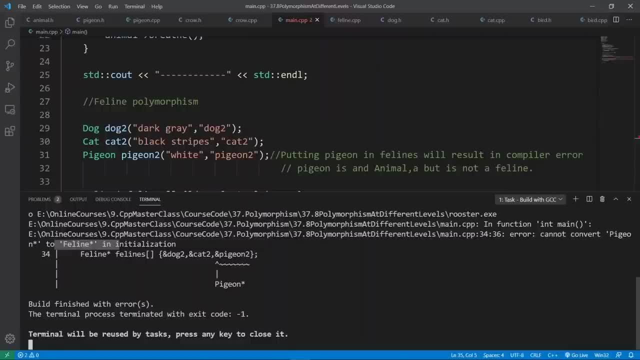 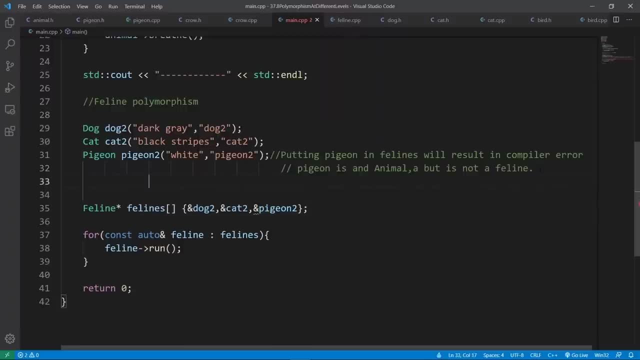 cannot convert pigeon to feline pointer. so this is the error here. you can't do something like this. even if you create an animal object, let's say that we're going to go in and create animal and we're going to say animal one, we can do that and we're going to pass in the description. i think we can do. 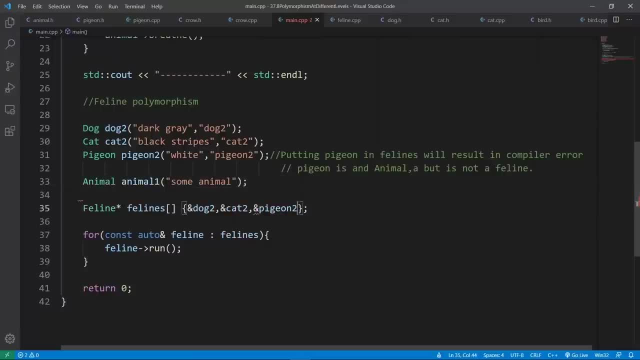 that we can do something like this, and if we try and pass in the address of animal one, let's do that. this is also going to give us an error and we're going to say animal one and we're going to also going to give us a compiler error, because animal is not a feline. again, if you get confused, 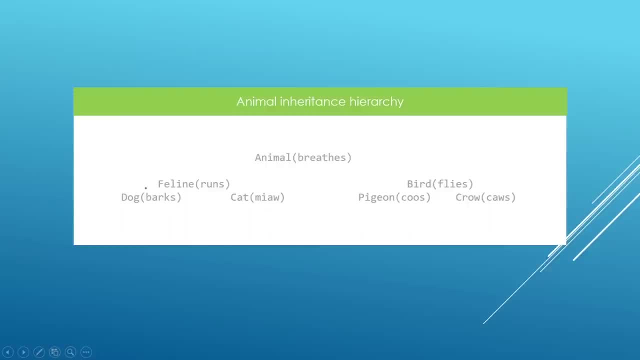 come back and look at our inheritance hierarchy here, what we are setting up in our code. we are using feline polymorphism but we want to store an animal in a rate that is storing felines, and this is going to be a problem because the compiler isn't really going to be able to process this. 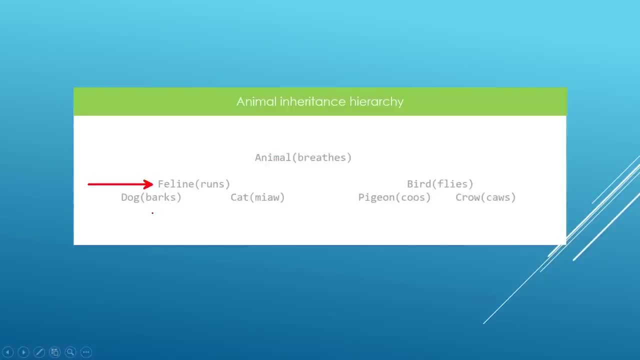 our base pointer is a feline and we should really be able to only store in derived types from feline. but we are putting in a super class or a parent class of feline which will not be able to have the specializations that feline is doing. so the 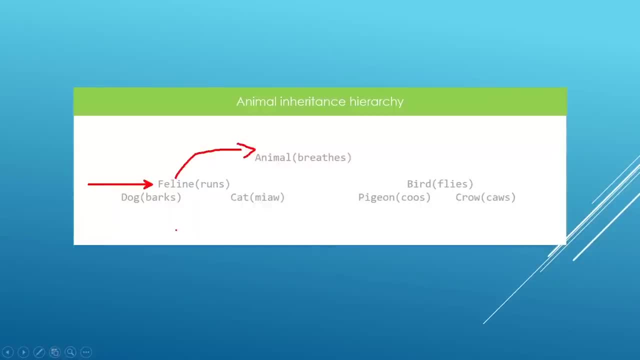 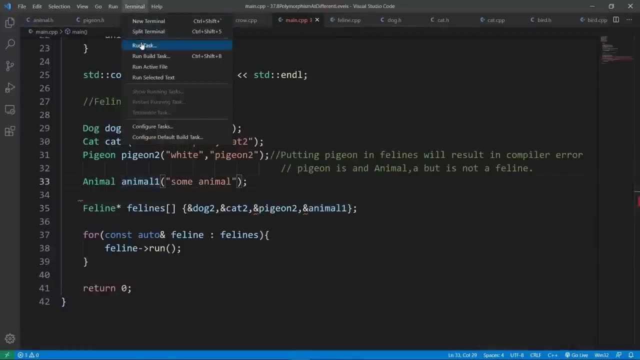 compiler is really saying: this is crazy, i can't do this. i am going to throw a compiler error. this is the behavior we get here. okay, so this is going to give us a compiler error and let's run and see that we're going to use gcc. the build is going to finish with an error and we are going to 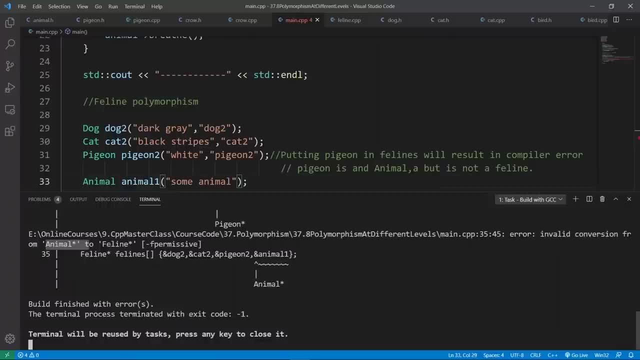 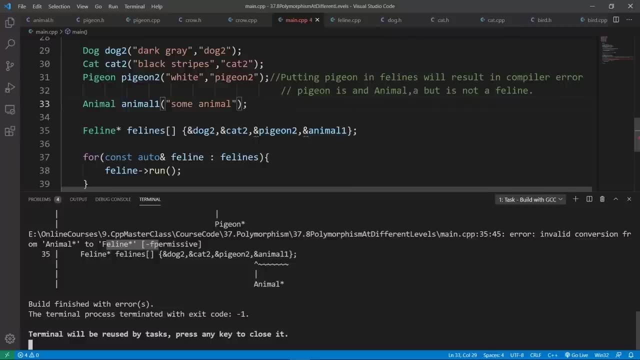 see that we have an invalid conversion from animal pointer to feline pointer. this is what we want to do here. we want to convert an animal pointer and store that in a slot that is only supposed to store feline pointers. so this is not going to work. but if you do everything right and only put in 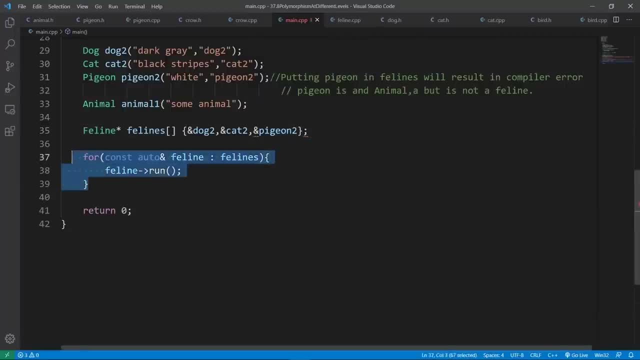 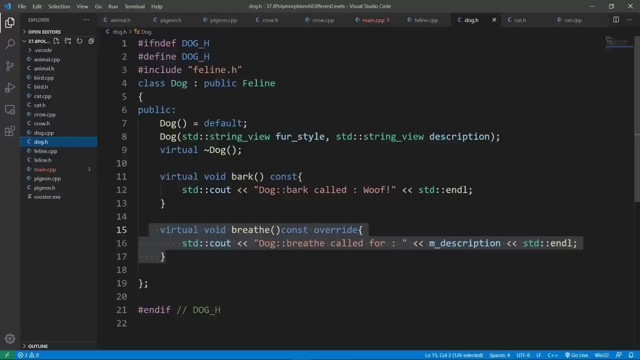 derived types of feline. you're going to get the correct length to work and let's look at our dog class. let's open it again. we're going to look at dog and we're going to have a run method, but we don't have that set up for our dog class. but we can do that. 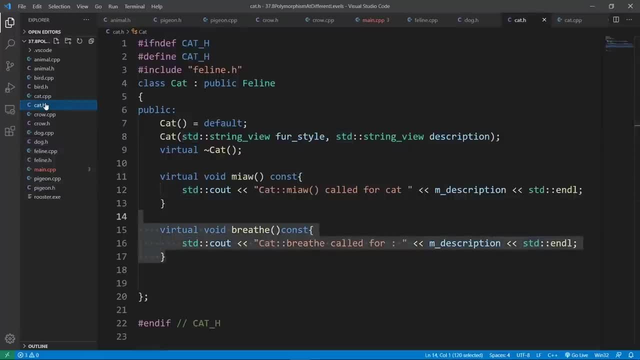 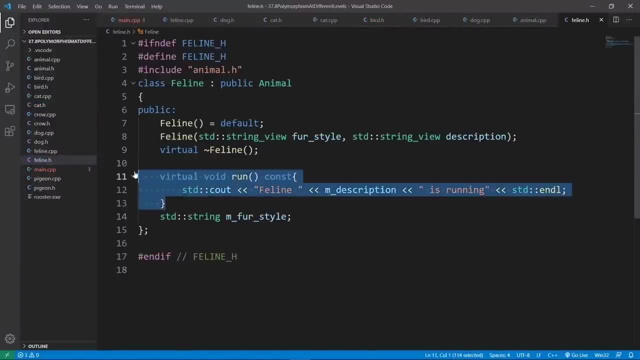 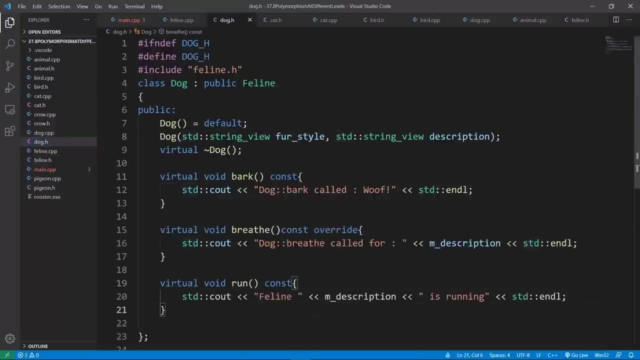 pretty quick. let's look at cat and see if we have a run method. we don't, but we can set that up. let's go to feline and copy our virtual function. we can do that and we are going to go in dog and set up another virtual method which is going to be run, and this is going to be an override of what we have. 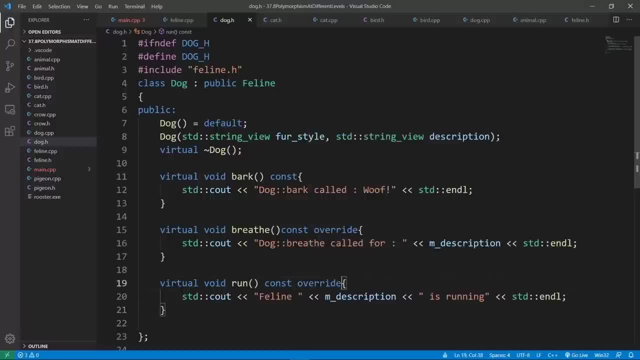 in our inheritance hierarchy, so this is an override method. we are also going to do the same, but before we go, let's say that this is the dog class we are doing things from. we are going to grab this method again and go in cat, because that's another feline we have in our program. 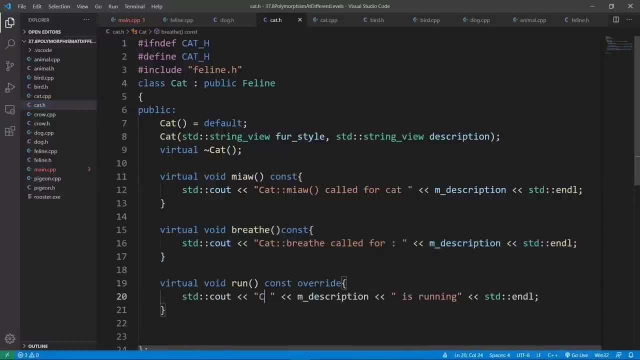 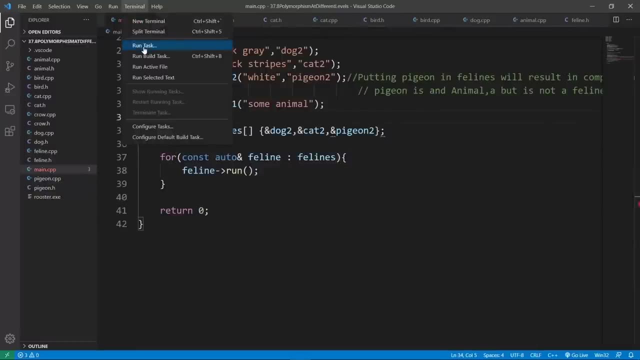 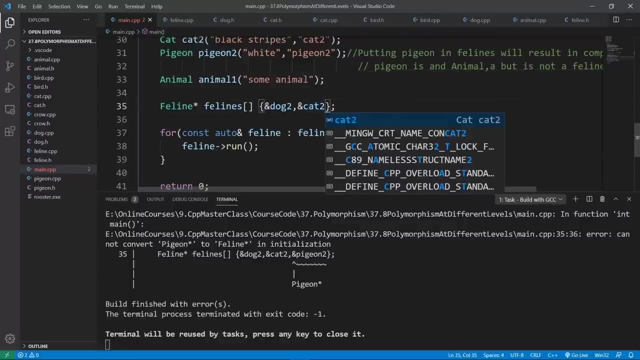 we can do something like this and we're going to say: cat here, okay. so now let's come back to main and we're going to build again. we're going to pass this through gcc and we still have a pigeon in here. so this is not good. let's take this out. make sure that we only have felines in this array. 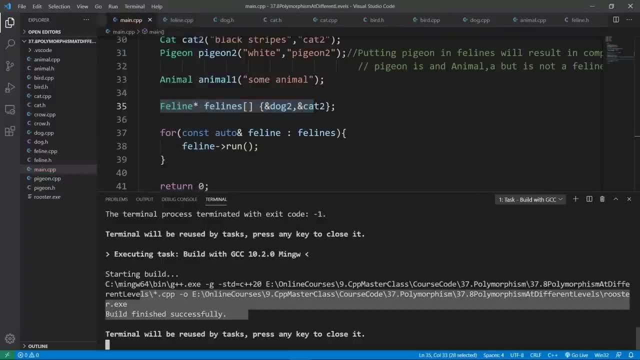 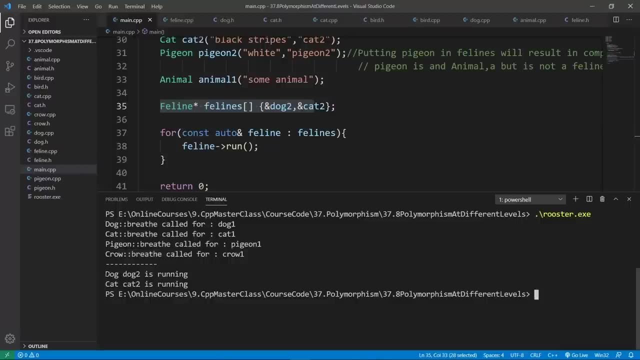 here, let's build again. okay, you see, the build is good, we can clear and run rooster. we're going to have our separator here and you're going to see that we are calling our dog method to the first iteration because the first object is a dog and we are calling a cat running method because the 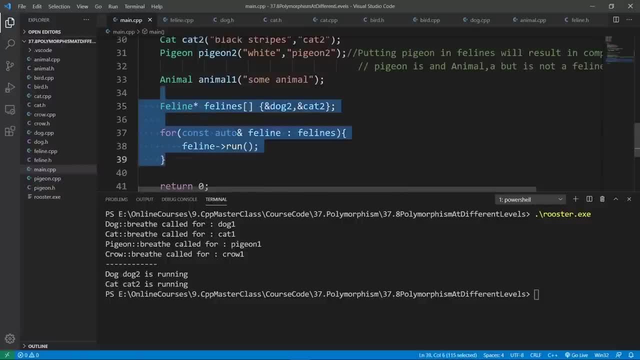 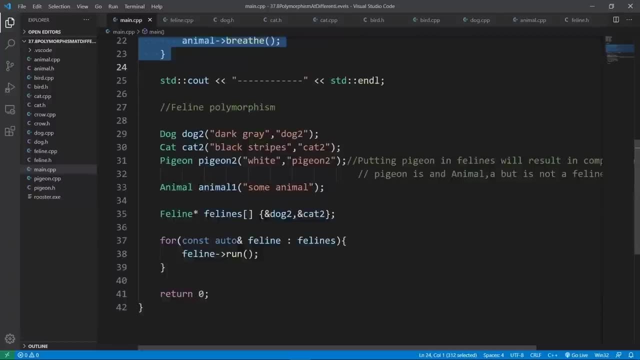 second object is a cat, and this is feline polymorphism in action. hopefully, this proves to you that we can do polymorphism at different levels depending on what we want to achieve in our c++ program. to close off this lecture, we are also going to set up 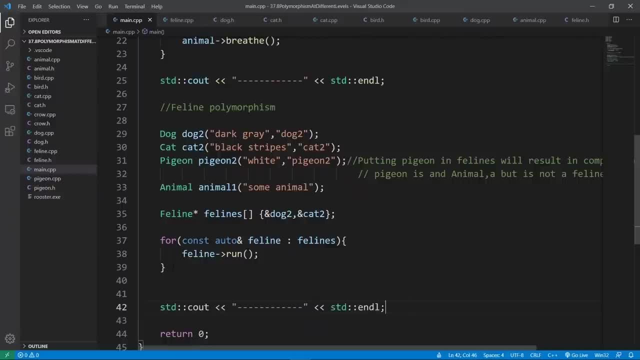 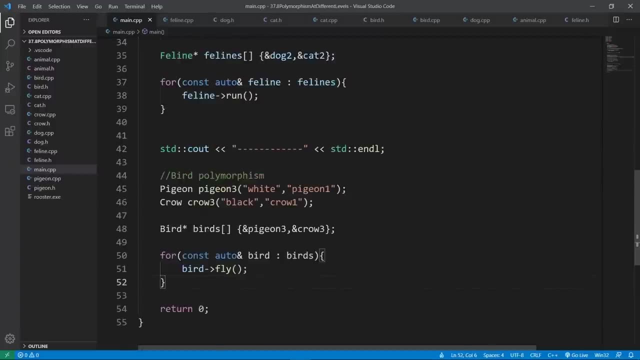 bird polymorphism. let's do that. we're going to put in a separator and we're going to say bird polymorphism, and we are going to put in a bunch of objects and set up a base pointer array, which is going to be a bird pointer array in this case, and we're going to be 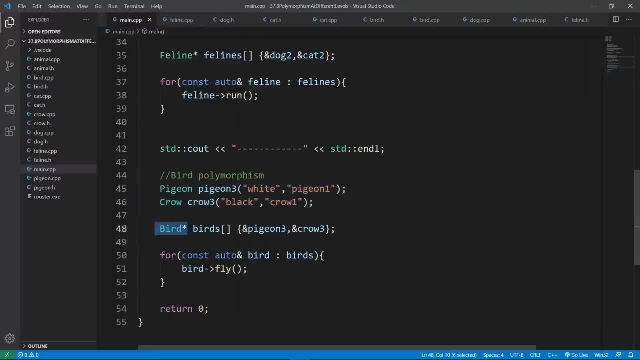 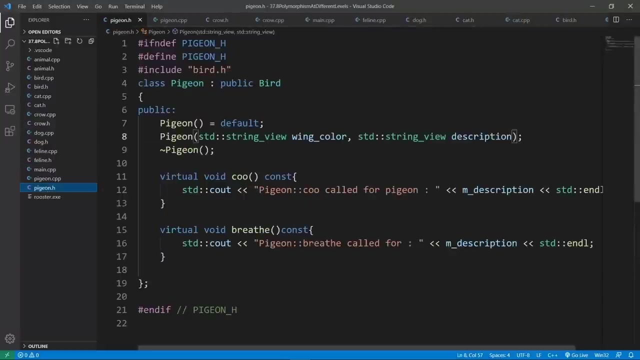 storing in derived objects of the base pointer type. so we are going to be storing in the derived objects of bird and we have a pigeon and a crow and this is the setup we want here. now let's go and look at the setup we have in our pigeon, for example. we don't have a fly method, we just have. 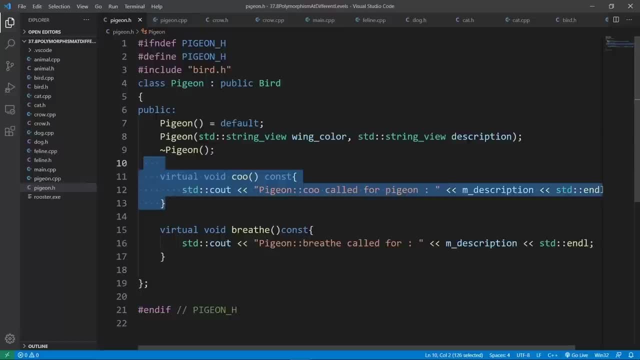 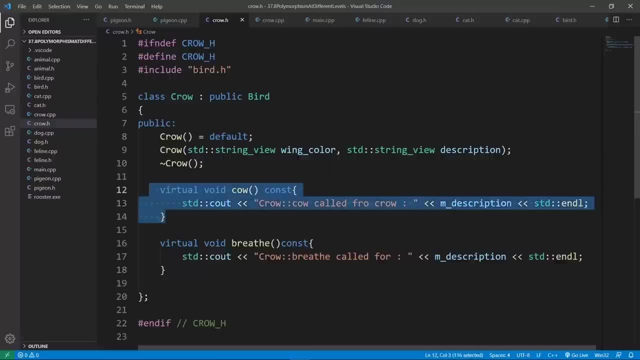 a coo method because a pigeon coos. if we go in our crow we're going to see that we don't have fly method. we just have in the cow method because a crow. but if we call our fly method because we don't have this method overridden in any downstream, 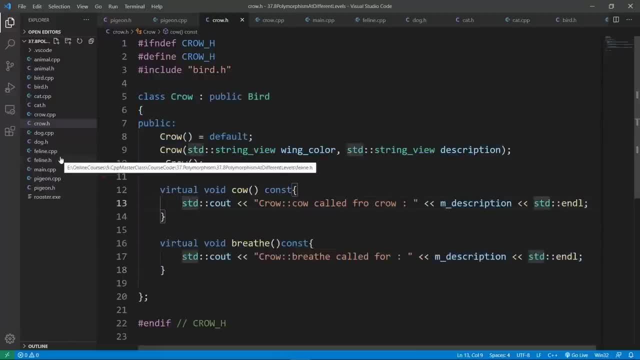 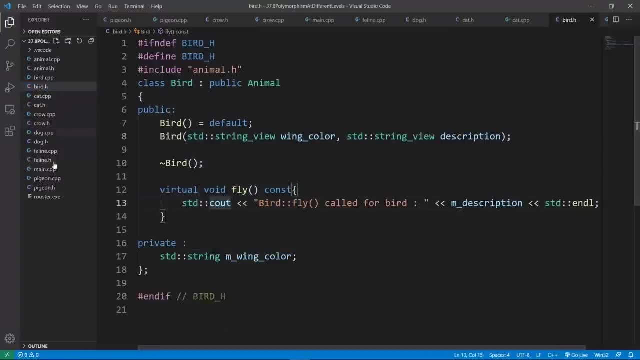 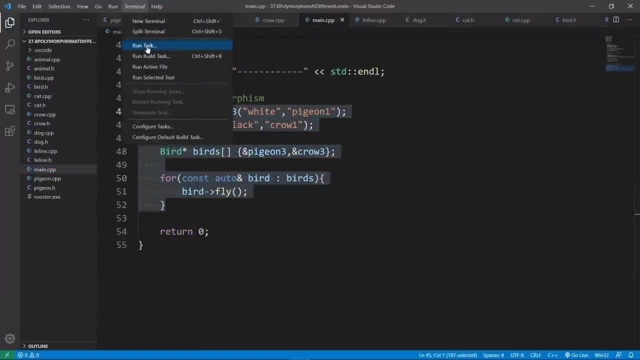 classes of bird. we will get the base version of the fly method called, so we will get this method here called. i want you to see this. let's hop over to the main cpp file and make sure we have the correct setup. looks like this is what we want. we're going to build this with gcc. the build is: 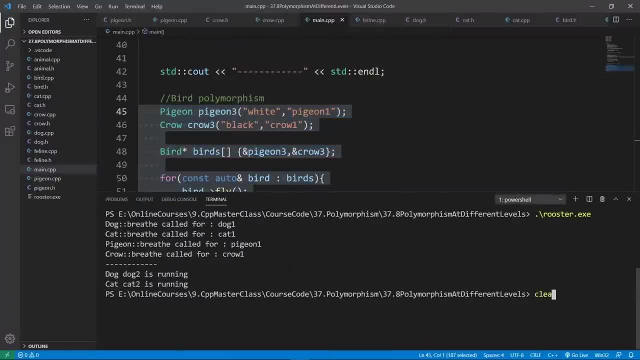 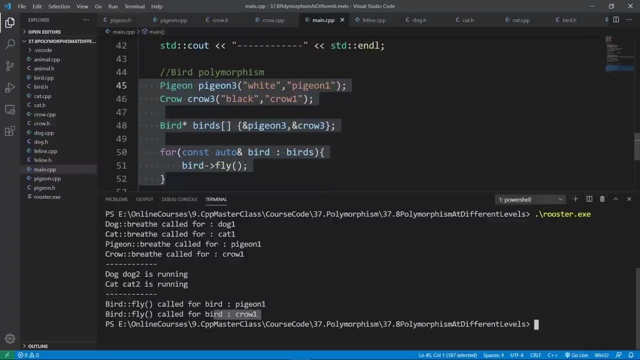 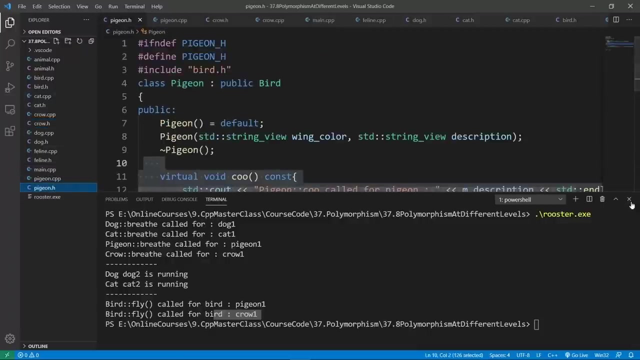 going to be good, as we see here, and we're going to set up a bird polymorphism and we're going to run. now we're going to see bird fly, bird fly for pigeon one and crow one, but this is not using any derived method that we have in our crow and a pigeon class. if you want, you can also override. 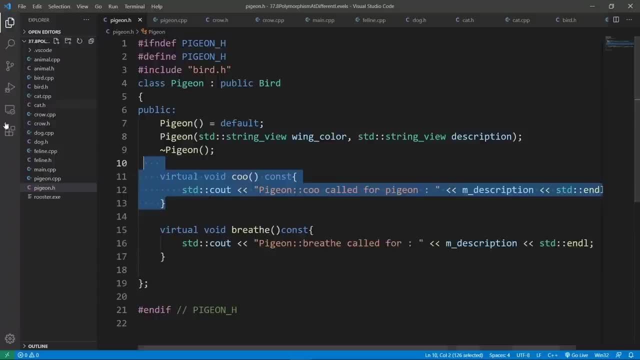 the fly method and you're going to get that called. let's actually do that because i'd like to show you things directly so that you can really see with your own eyes. so we're going to go in bird and grab the fly method and we're going to override the fly method and we're going to 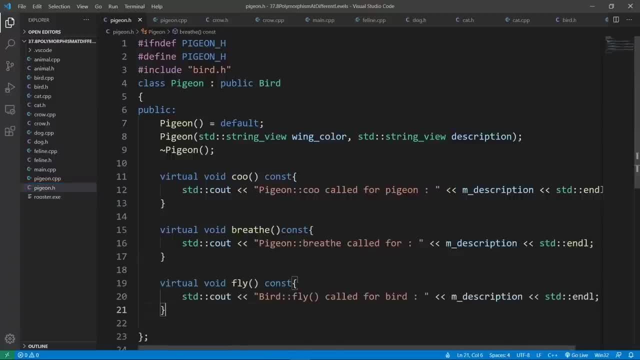 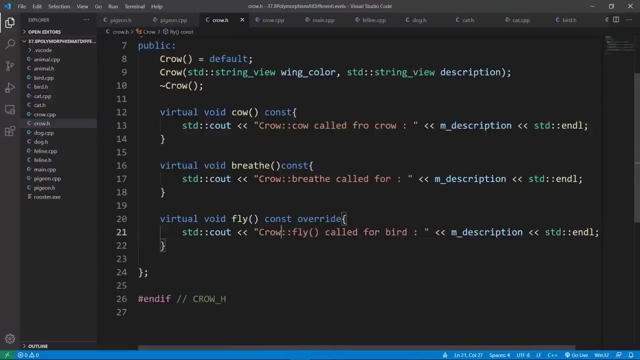 override this in pigeon. we can do that and we're going to override here and we are going to say pigeon here, and we can grab this and put this method also in the crow class. we can do that and we're going to say crow here. now, if we run this program using what we have in the main, cpp. 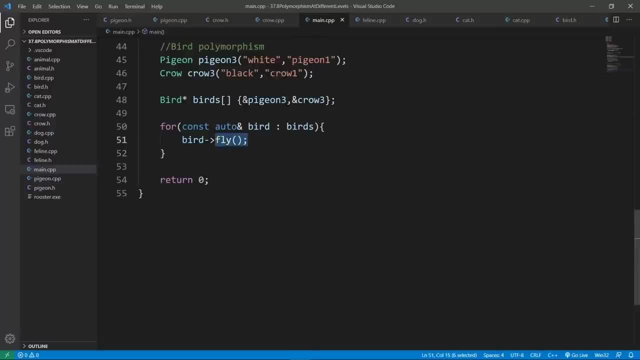 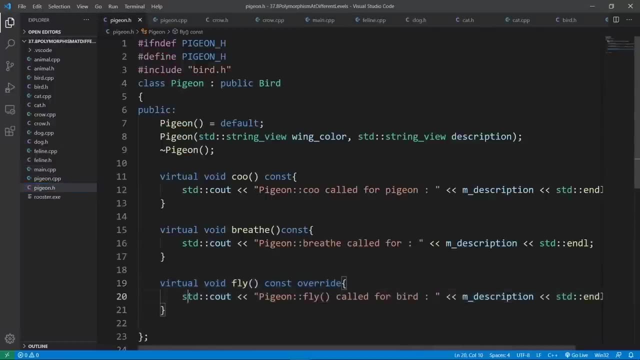 file for the first iteration. we're going to call the fly method on the pigeon object, because we have the fly method overridden at the pigeon level, as we see here. this is right here beneath our eyes and we're going to see this in action. if we run this program here, the same is going to 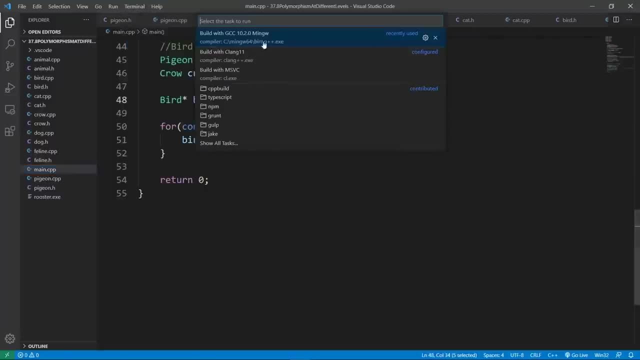 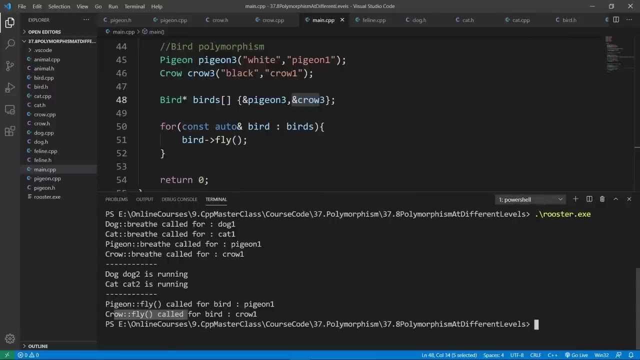 happen for the crow object here. let's build with gcc to really prove this. the build is going to go through. we can clear and run rooster and we're going to see pigeon fly, crow fly. this is proving what we set up in this lecture here. this is really all i had to share. i hope you found this. 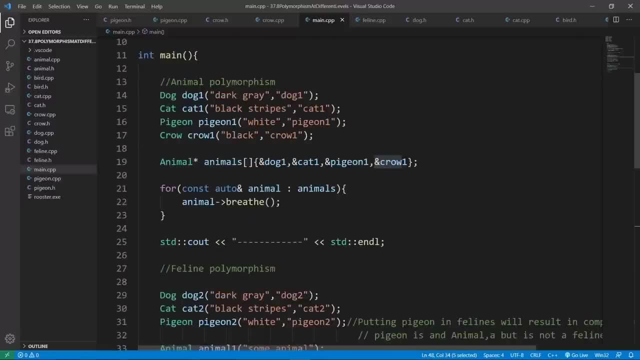 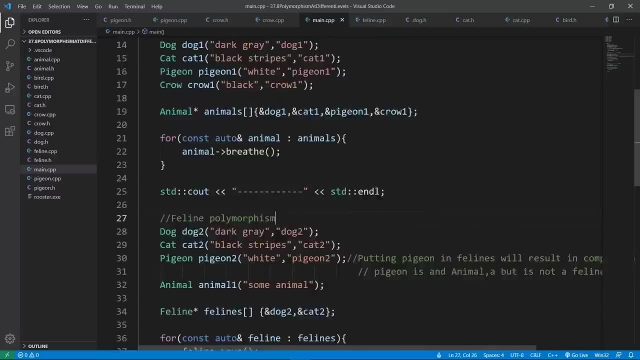 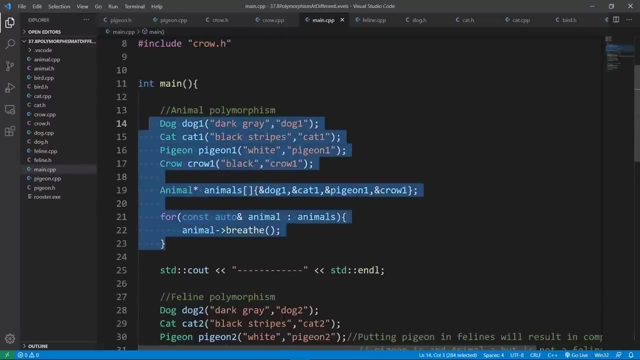 interesting. the main message is that you can set up polymorphism at different levels in your inheritance hierarchy depending on what you want to achieve. in your c++ program, we saw that we could do the usual thing and use the top level class as the driver for our polymorphism, and we did animal polymorphism here, but nothing. 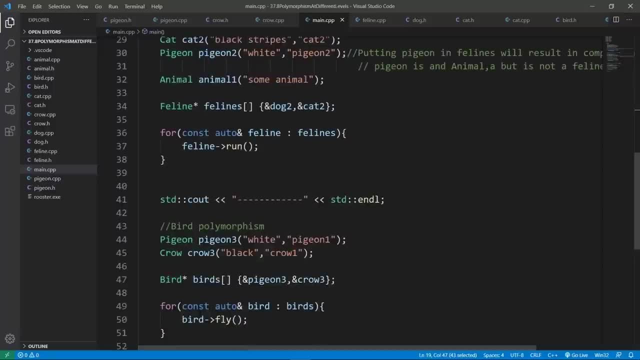 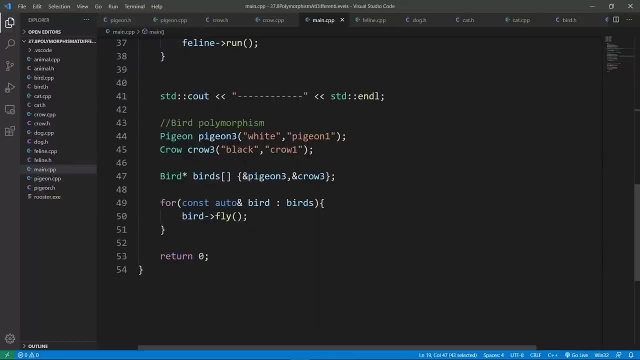 prevents you from doing feline polymorphism or bird polymorphism, as we saw in this lecture. we are going to stop here in this one. in the next one we're going to see how we can do polymorphism. in the next one, we're going to see how we can do polymorphism in the next one. 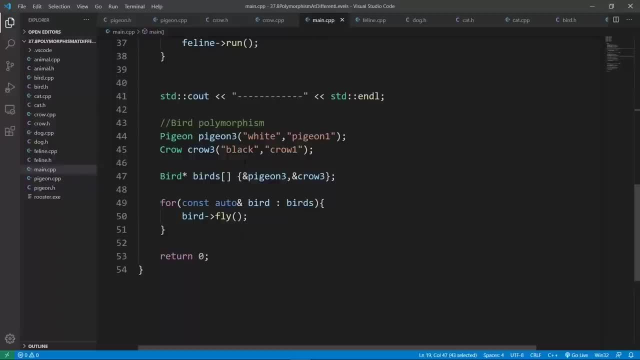 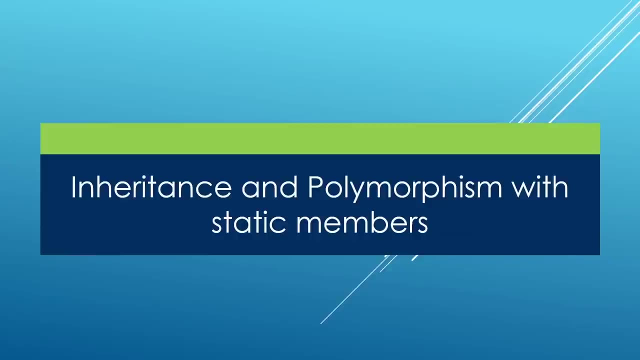 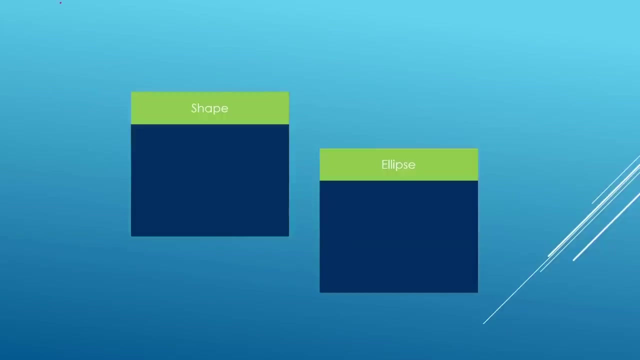 polymorphism with static members. go ahead and finish up here and make me there. in this lecture, we're going to explore how inheritance and polymorphism play out with static members that we have in our classes, and we're going to be using this inheritance hierarchy here our base. 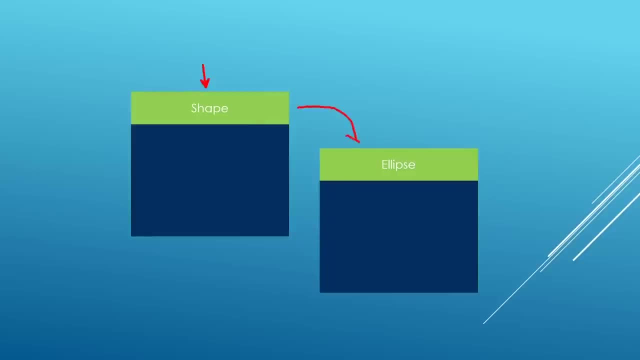 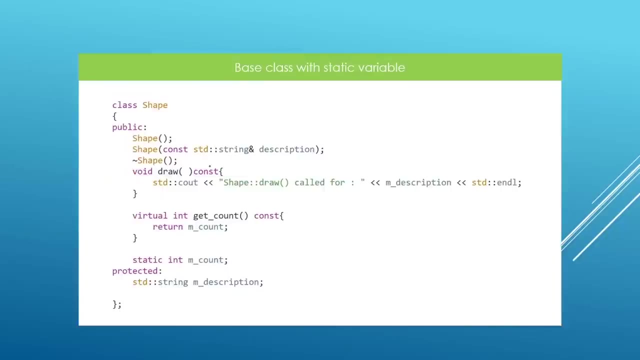 class is going to be shape. we're going to inherit from that and create an ellipse class. let's look at some code here. so we're going to set up our base class as a shape, as we said, and we're going to have one member variable which is going to be our description here. 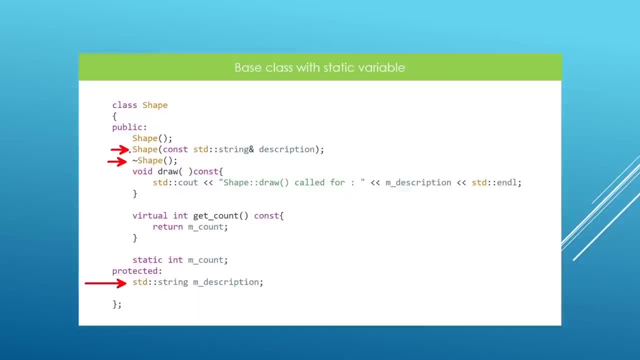 we're going to have a constructor and a destructor and we're going to have a default constructor, which is really not important here. but notice that we have a static member which is called m count and, if you remember, a static member variable is a kind of variable which is associated with the 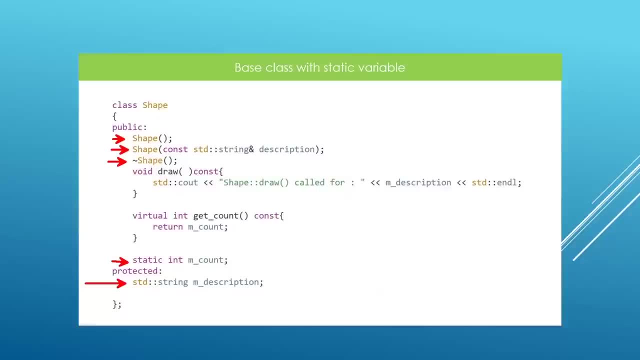 type itself. it's not associated with any object that you create. if you forgot this, please go back to our chapter on classes or user defined tabs. you're going to learn all about static variables here. we are just exploring how they play out with inheritance and polymorphism. 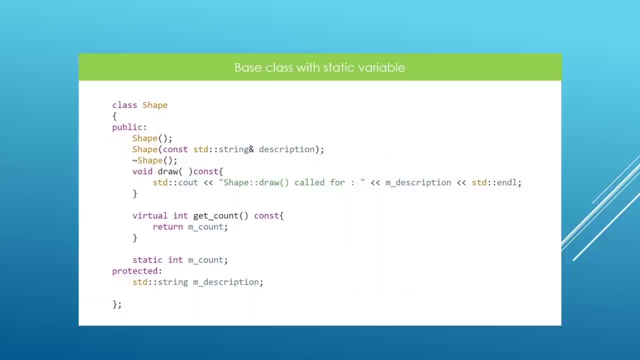 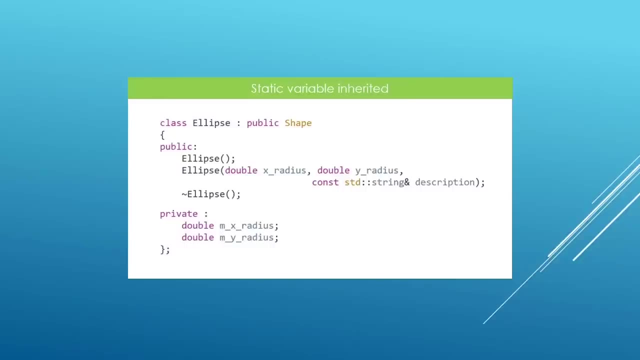 now we have a shape class. if we inherit from it and create an ellipse class, for example, we're going to have all the data that was public in our base class to be public in this class as well. so by that logic, we are also going to get this static variable inherited and we're going 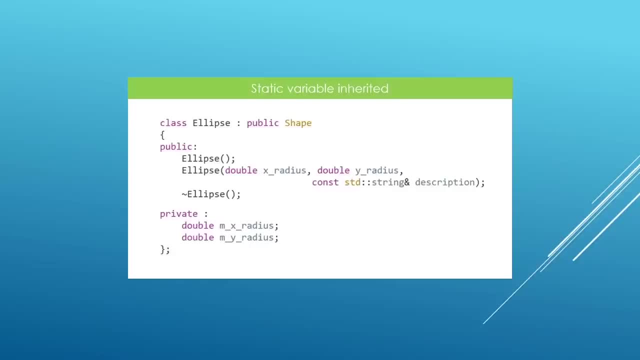 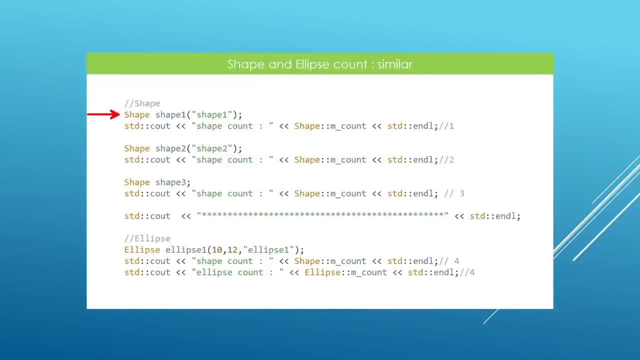 to be able to access it from ellipse objects. let's try and use this in code here to really drive the point home. here we are creating a bunch of shape objects. here is our first shape. we print our static variable through this syntax here, because it is public, we can do this. we're going. 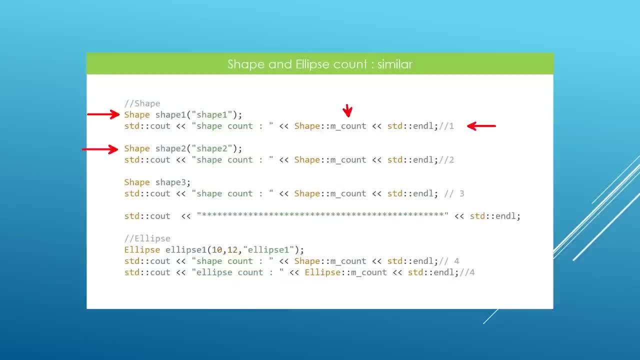 to get a one because we just have one shape here. we create a second shape and we print the count. we're going to get two because we just have two shapes in here. we create our third shape and we try and print the count. we're going to get two because we just have two shapes in here. 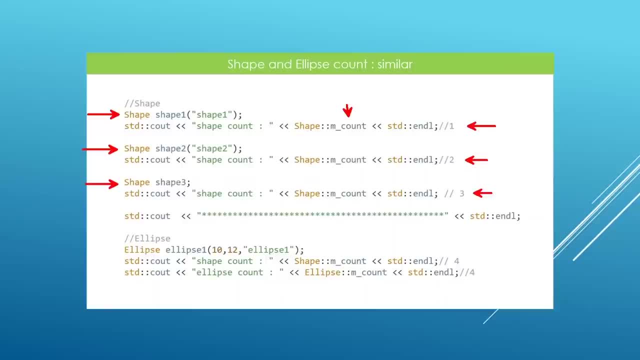 to get three. and if you wonder how we are incrementing this static variable, we may do this in our constructor. we're going to see how this works exactly once we hit visual studio code in a minute. but note that every time we create an object, we're going to be incrementing our static 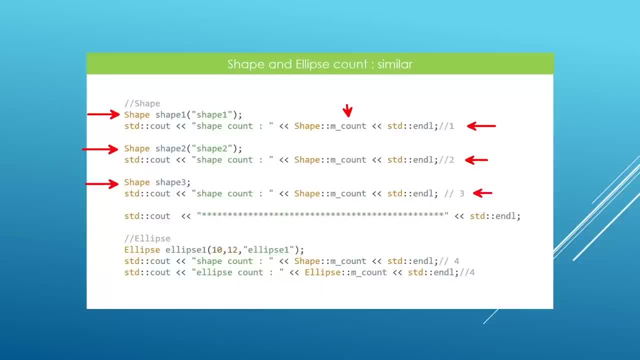 variable. that's why we see one, two, three as we create these objects here. this is the logic. now we have three shapes here. we go down and create a new object which is of ellipse time. if we print the shape count, we're going to get four because we're going to get three, and if we print the 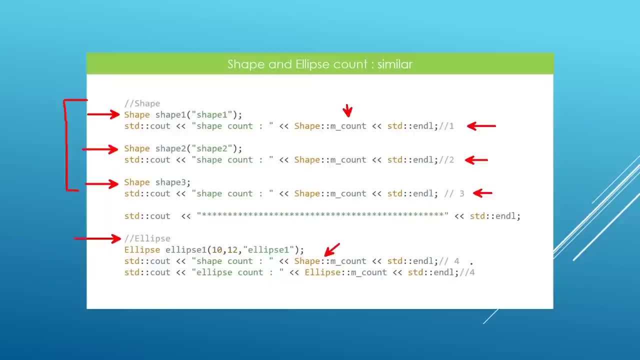 ellipse count, we're going to get a four, even if we really just have one ellipse. so the static variable from shape is being inherited and used in our ellipse class, and this may not be what we want. so the problem here is that the static variable we are using in shape and ellipse 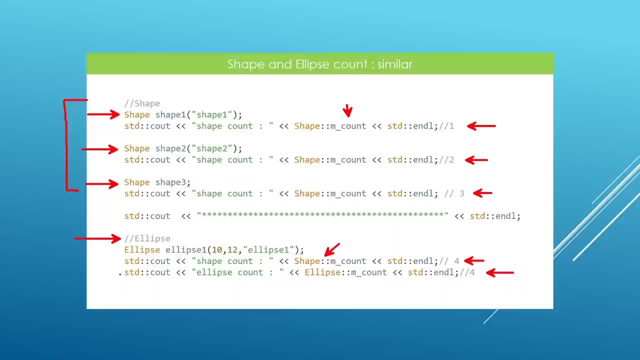 are the same, because the one we have in ellipse was inherited from shape. that's why we have these results here. but sometimes we just want to have ellipse count to be one here, because in reality we really have one ellipse. so how do we do that? to get that behavior, you can also set up another. 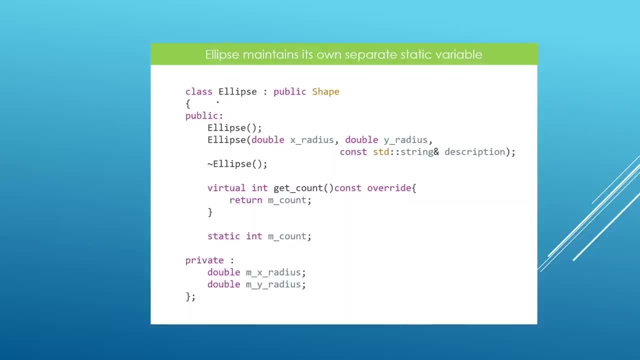 static variable named exactly the same way at the ellipse level and you can do that like this. you can also override the get count method to return the current count in the form of the static in ellipse. this is going to work through polymorphism because the get count method 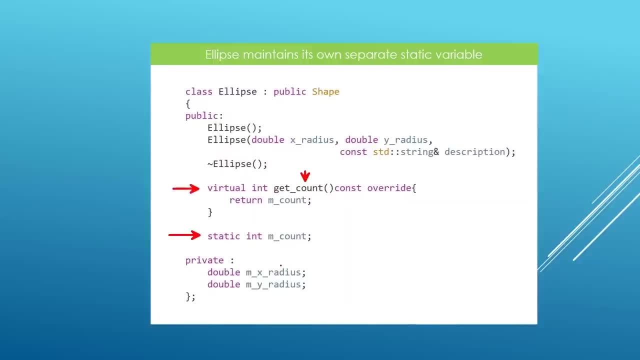 is a virtual function. if you call this method through a base pointer, you will get the correct one called, which is going to be the most specific one through polymorphism. but what we want to see is how things are going to work now that we have a static variable which is named exactly the same. 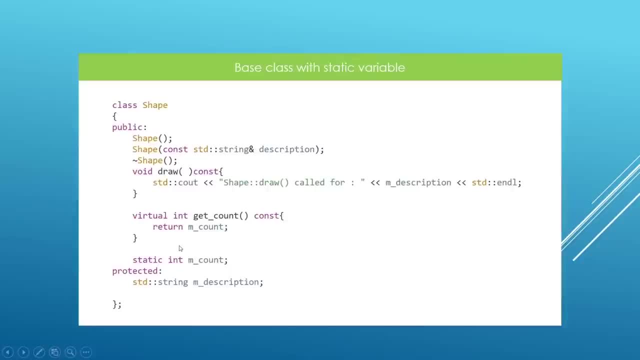 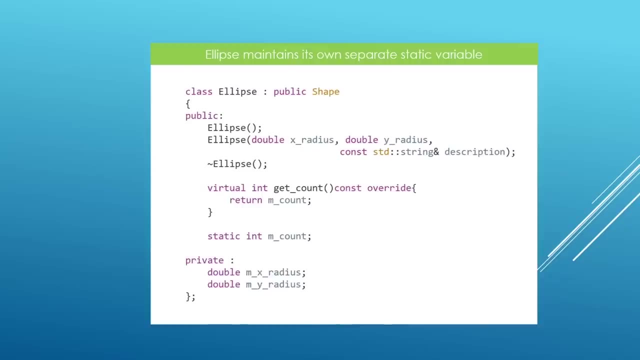 as the one we have in our base class. here, the one in shape is exactly named m count. it is a static variable of type, and the one we have in ellipse is also the same. it is a static variable called m count of type. and but now ellipse is going to maintain its own static variable. 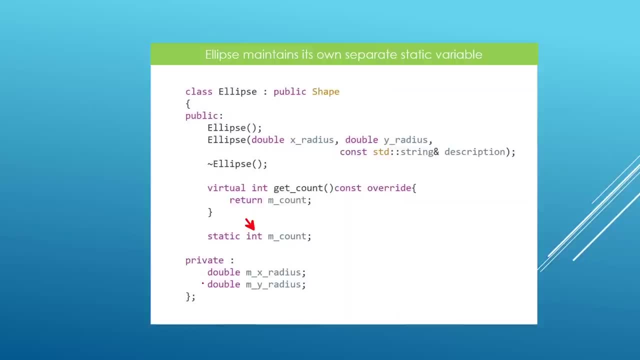 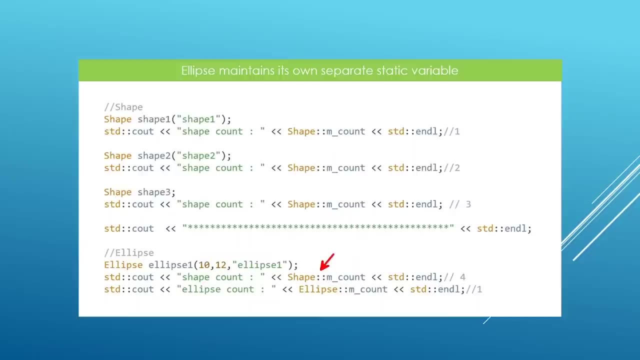 and shape is going to maintain its own static variable. now we are going to get this kind of behavior. we are going to see that if we try and print the count of shapes we have, we're going to get a four here. but now, if we try and print the count from ellipse, we're going to get a. 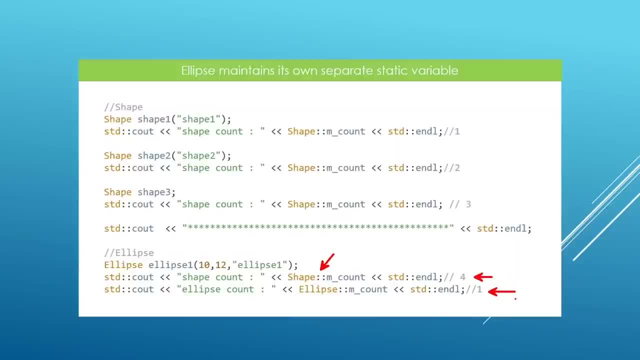 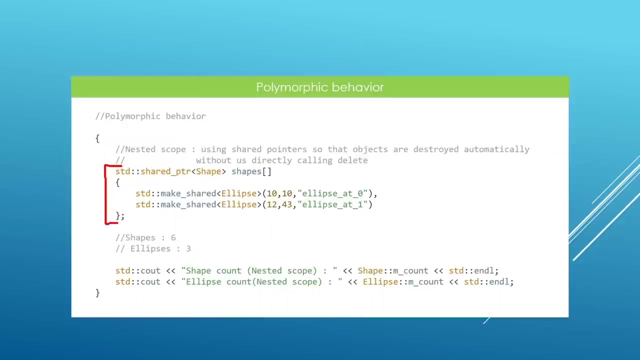 because we really have one ellipse and this is working because ellipse is going to maintain its own static variable and this is going to give you this behavior, if it is what we are after in our c++ program. now we can also go on and create a bunch of other objects. here we are going to 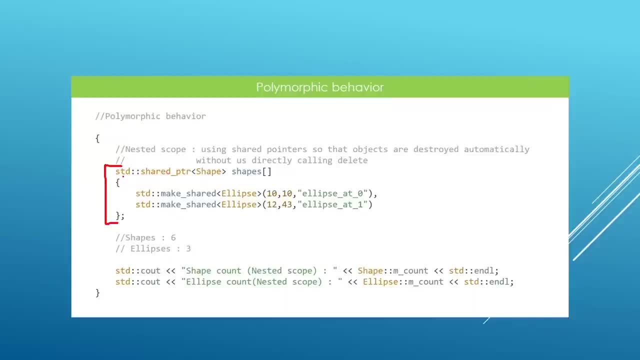 store them in this array, which is going to be storing shared pointers to shape, and we're going to store in derived objects. this is the syntax we can use to do this and at the moment we do this, we're going to get six shapes, because in total we really have six shapes, but three of. 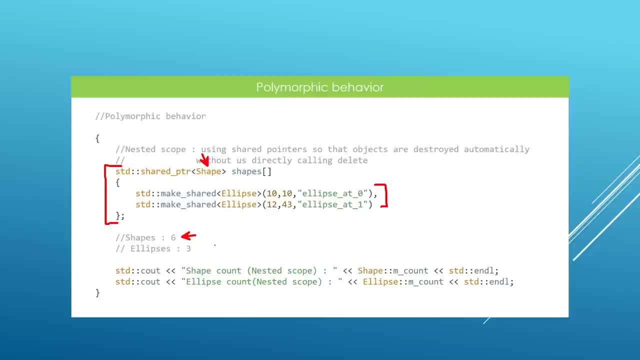 those shapes are going to be ellipses and if we try to print the ellipse count, we're going to see that we have three ellipses in our c++ program and this is going to do what we want. another thing you could do is also do shape polymorphism and call the get count method and you're going to get. 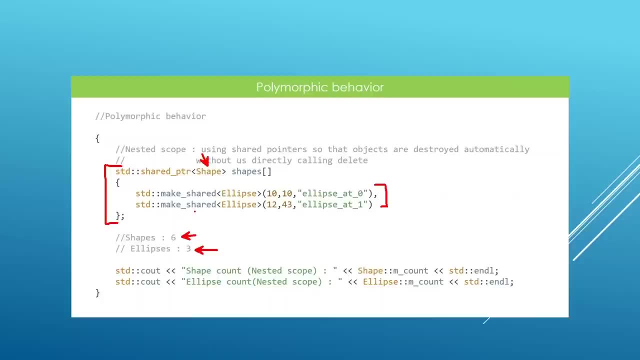 the correct to get count method and print the most specific count. if we are calling that method on an ellipse object, for example, we're going to print three. if we call that on a shape object, we're going to get sex. and that's the behavior we could achieve with polymorphism, with 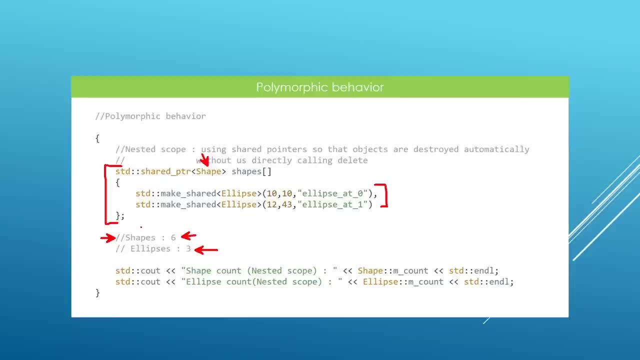 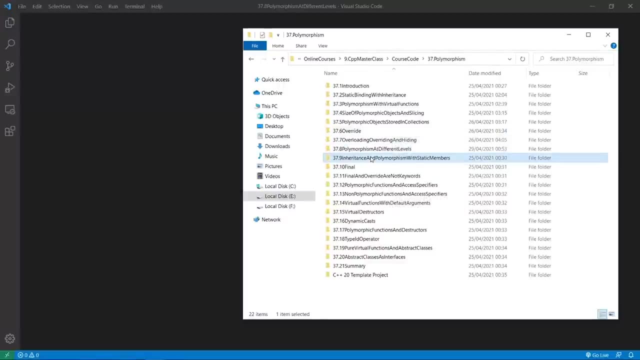 static member variables, and i really want you to be aware of this. now that you know this, we're going to head over to visual studio code and play with us a little more. here we are in our working folder. the current project is inheritance and polymorphism with static members. we're going to grab our 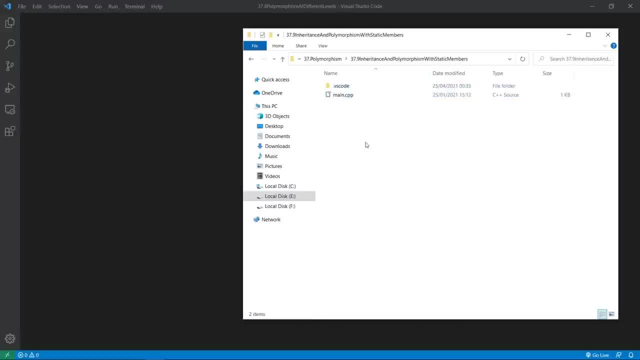 template files and put them in place, and i am going to grab our classes from my drive and use these as the starting point. again, if you don't want to type or create these classes, you can use the files provided in the resource section of this lecture. you can download them and use them directly without having to create them, because we 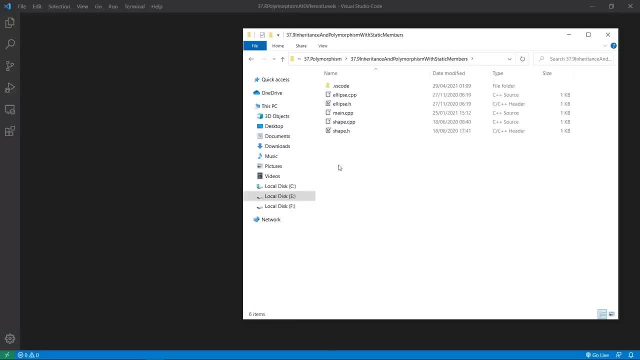 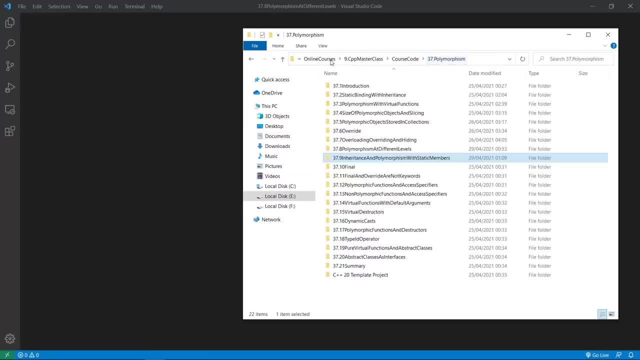 are really interested in how static members behave with our inheritance hierarchy, which happens to be setting up polymorphism. this is what we want to learn about here. i am going to open this up in visual studio code and we're going to take a good look at our classes. the 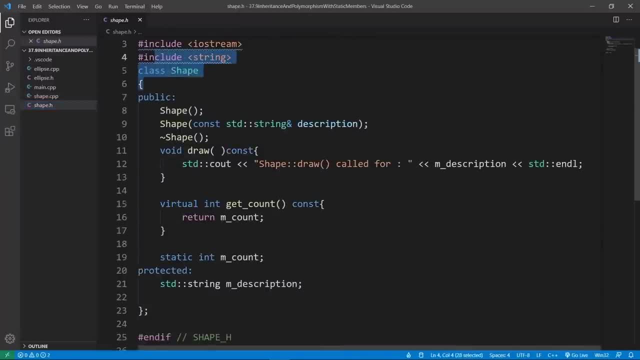 base class is going to be shape, which is what we have here. it's going to have a virtual method, which is get count here, and we have a static member which is of type int. i am going to change my parameter here to be std string view, because that's what we should do in modern c++. let's look. 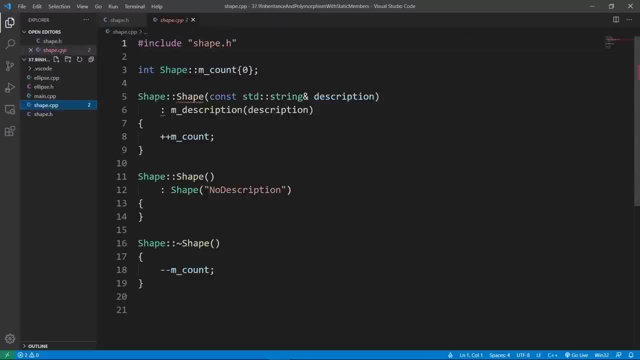 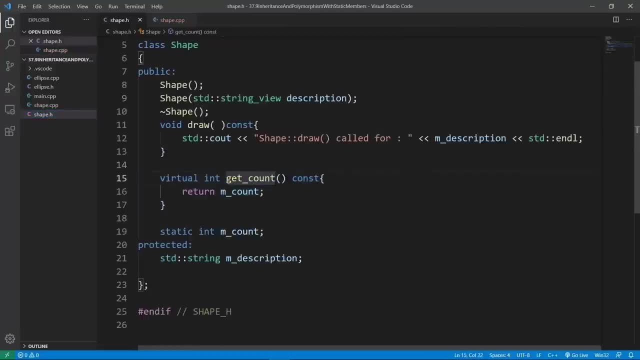 at the cpp file for this and we're going to fix this a little bit and we're going to hop over back to the header file and look at what we have. we have a virtual method which is going to return this count here. it is a cost method because it's really not going to modify, it's just going to 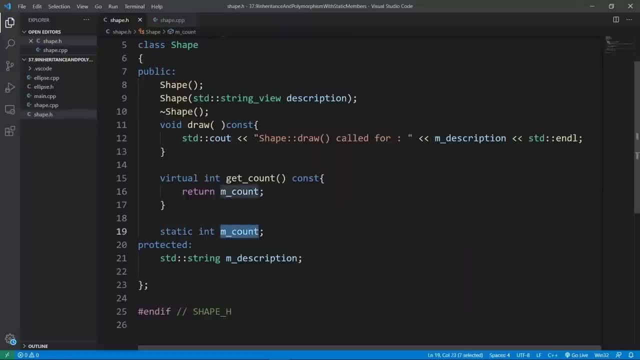 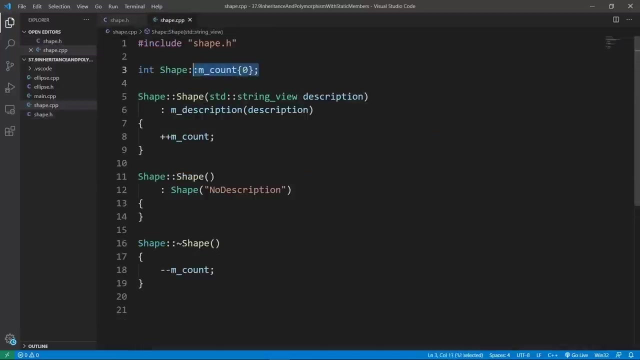 return a copy of the count member variable we have here and this is a static member variable. notice that it is not in line. so we will need to define this in the cpp file somewhere, because this is a declaration. we need to put in a definition, which is what we have in our cpp file here, because we 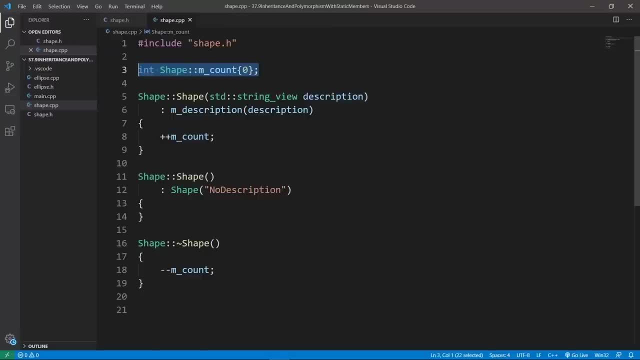 need to define this in the older c++ way. we are going to increment our account member variable in our constructor and this is going to achieve the behavior we really want: to have the m count member variable, which is static, incremented each time. we'll create a shape object here. 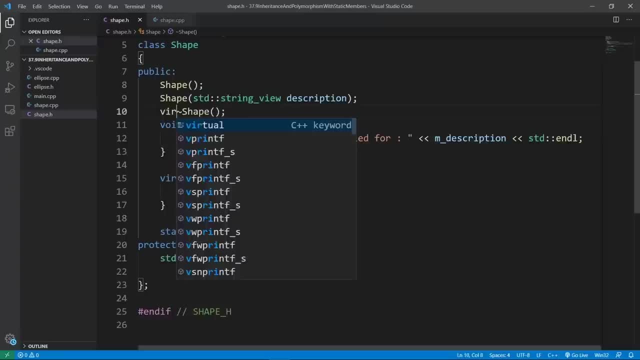 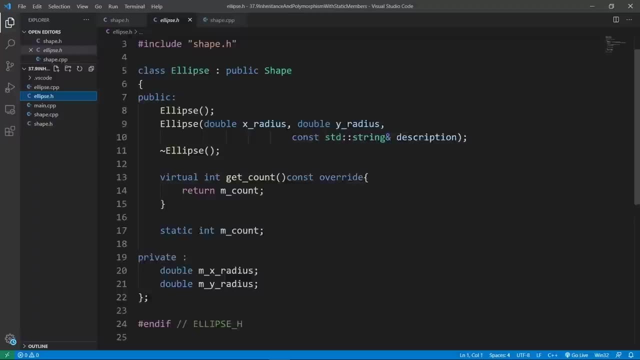 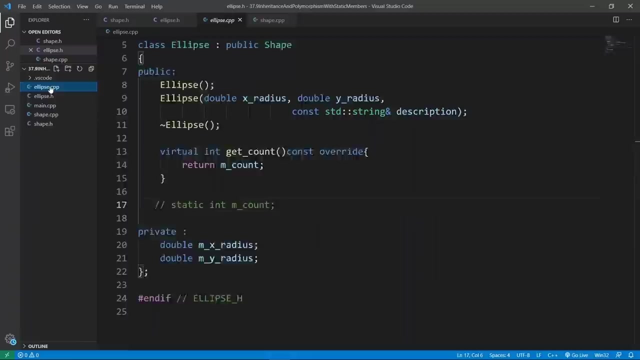 let's go back and look at our destructor and make sure that it is virtual, because we have virtual functions in this class and this is the setup we have. let's look at ellipse and we're going to take static member variable because we don't want to set it up as of now. we will enable it in a minute. 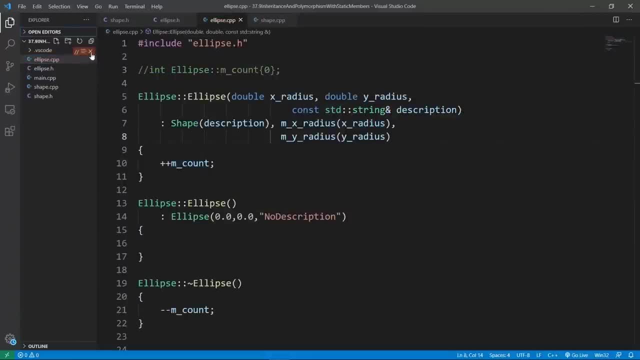 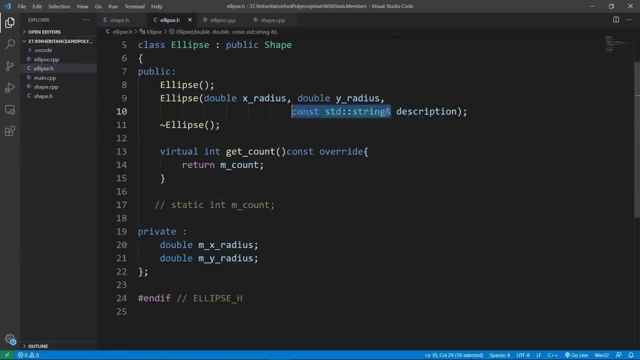 let's make sure we remove this and let's remove this, because i don't want this. and now we can try to create objects of our classes and see how these guys play out. we can also go in ellipse and make sure the constructor is taken. std string views. where we are needing strengths, we can do. 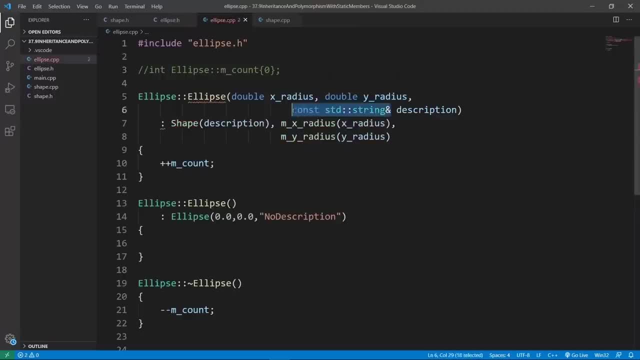 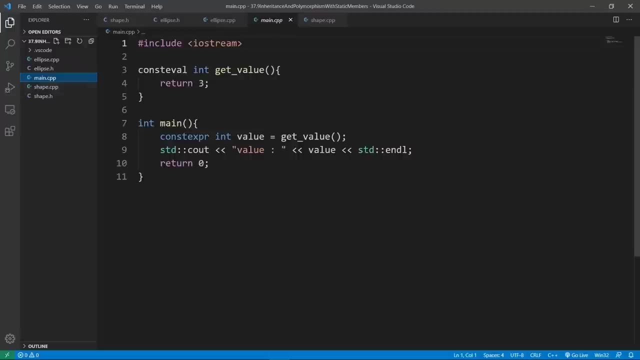 that and uh, hop over here and we're going to create a new class and we're going to create a new class to the cpp file and do that std string view. i think this is going to make visual studio code happy. by now we can hop over to the main cpp file and clean it up a little bit, and we are going to 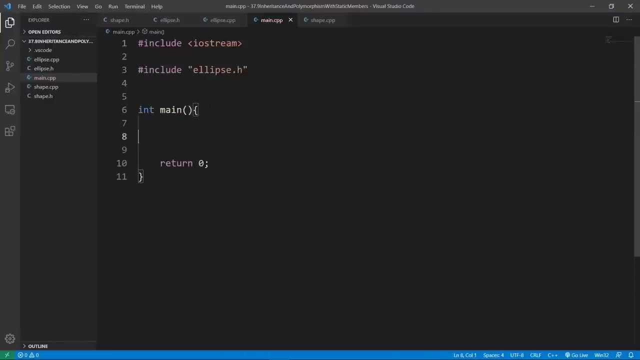 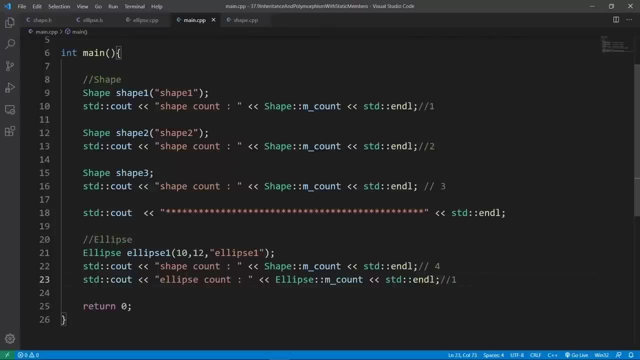 include ellipse and in our main function we're going to create a bunch of objects. let's close the left sidebar here, because we don't really need that anymore. we're going to create a shape object and we're going to print the shape count. we expect to get a one, because we just 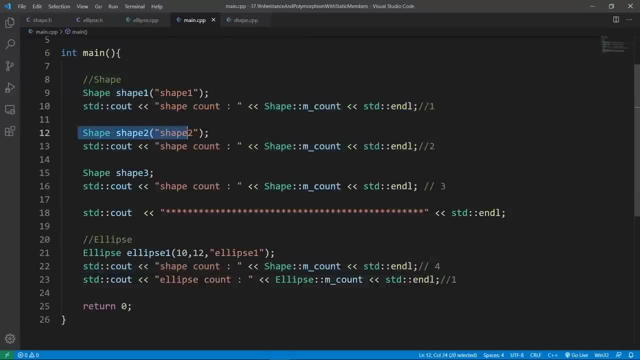 have one shape at this moment. we're going to create a second shape here and if we print the count, we're going to get two, because we have two shapes. this is what we expect. we create another shape, which is going to be shape three. here, we print the account, we're going to get a three. 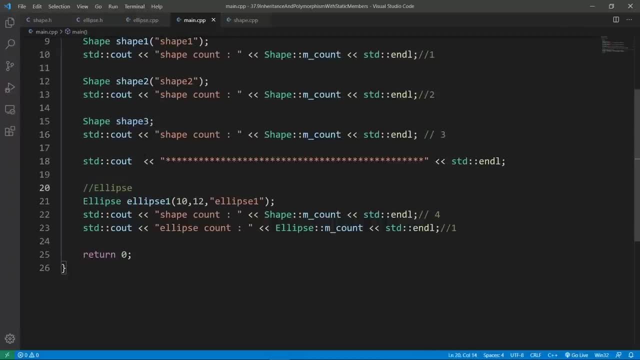 but the problem is going to come when we create an ellipse here. if we create an ellipse and print the count, we're going to get a four, because we have four shapes in our c plus plus program. but if we print the ellipse count here, we expect to get a one, but that's not what we're going to get. 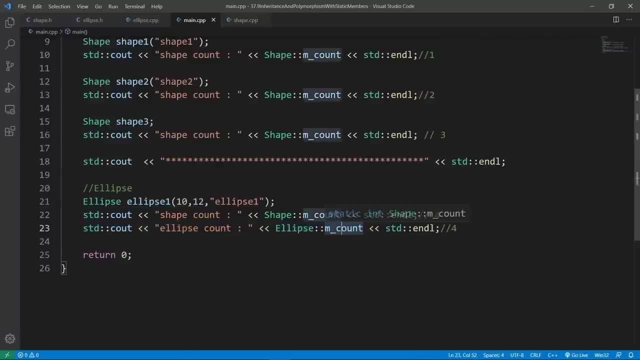 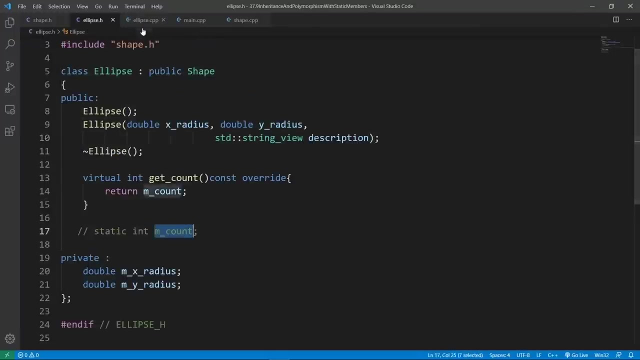 we're going to get a four because the m count variable in ellipse is inherited from our shape class, so it is going to be the same thing we have in shape here, because if you go back you're going to see that at this point ellipse doesn't have a static variable- m count- of its own, so it's going. 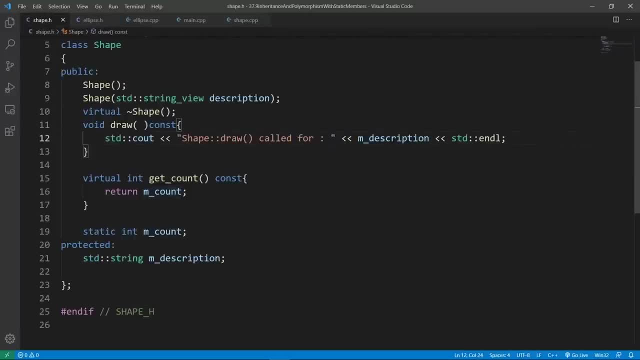 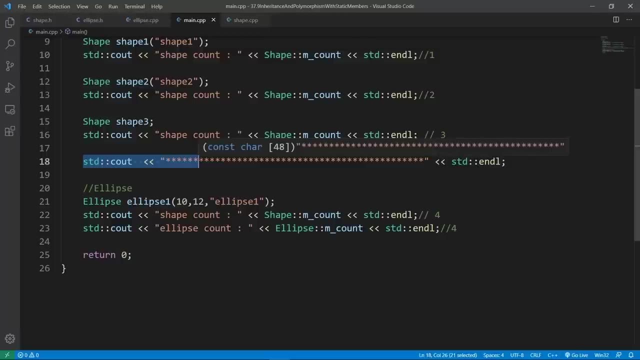 to use the one it is inherited from the shape class. this is the behavior we're going to get here, and i want you to be aware of this. if this is what you want, this is fine, but in most cases, you will want this to be different, because you want very clear information about how many objects 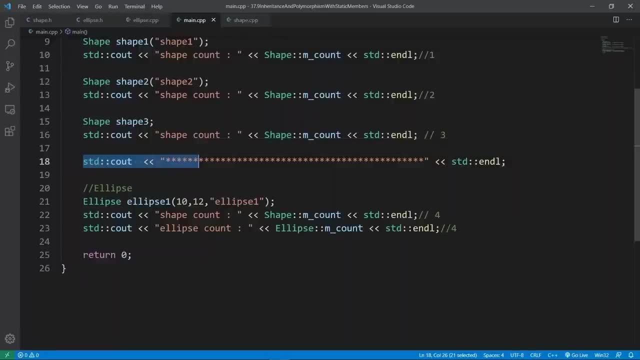 of each type you have created in your c plus plus program. if it is just shape, this is going to be really vague because you want to know if it is an ellipse, if it is a rectangle, if it is a triangle. this is not going to be super clear, so let's weld and really show you the problem. here we're going. 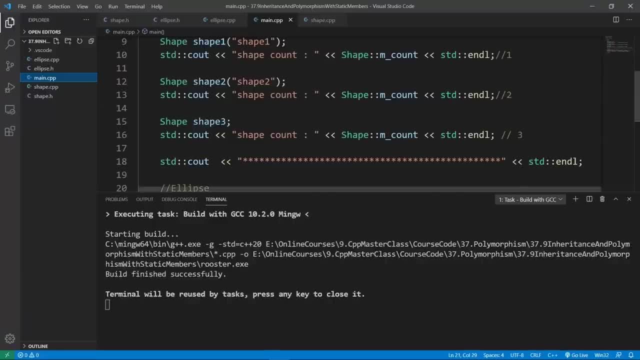 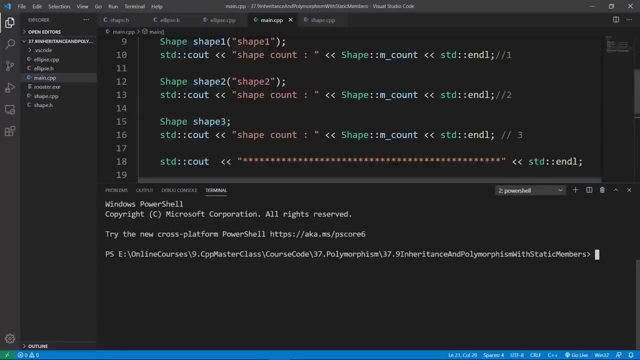 to pass this through gcc, our favorite compiler. we can also bring up the left sidebar- no problem here- and we're going to bring up a terminal window or a powershell window. i can say: we're going to clear and run rooster, you're going to see that. 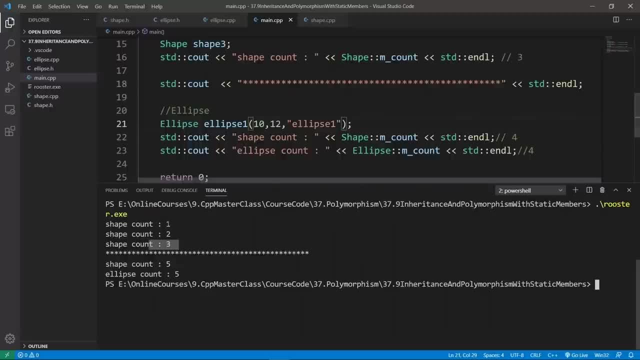 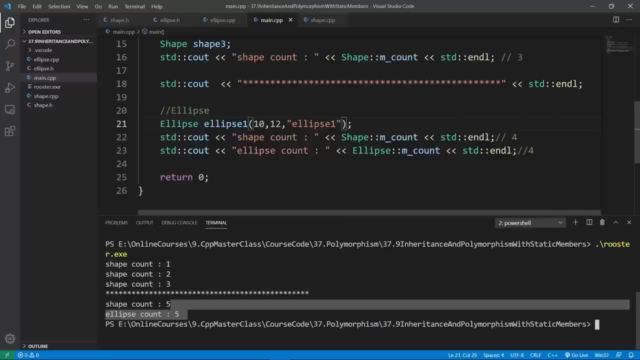 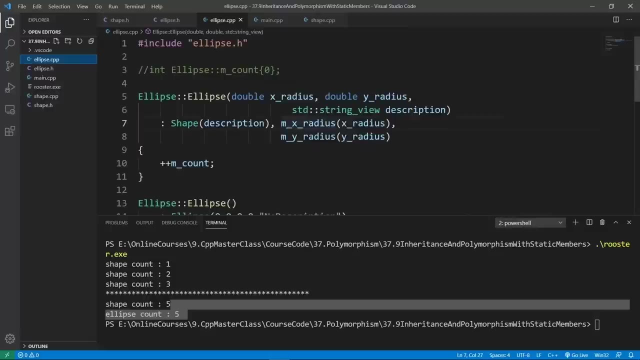 the shape count is going to be one, two, three and we have a five here, because we are also incrementing the m count variable in our derived class. so we are incrementing twice. if we create an ellipse object, let's show you this: in ellipse cpp, we are incrementing the m. 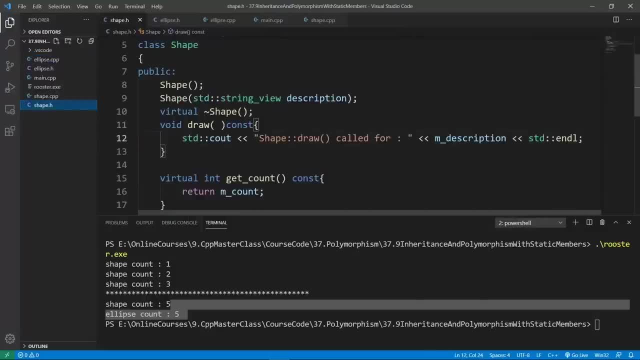 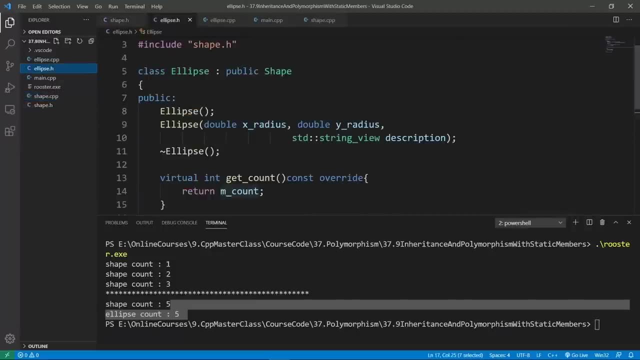 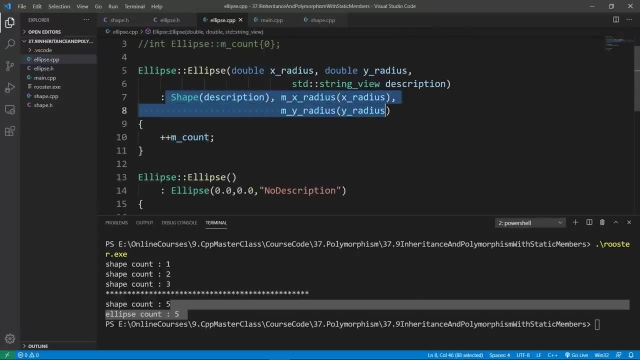 count member variable, but in the base class we are also incrementing that in the cpp file- that's what we have here- and notice that the derived class is also calling the base class through our initializer list here. so this is the behavior we have. we shouldn't be incrementing this, because ellipse doesn't have its own static variable as of now. 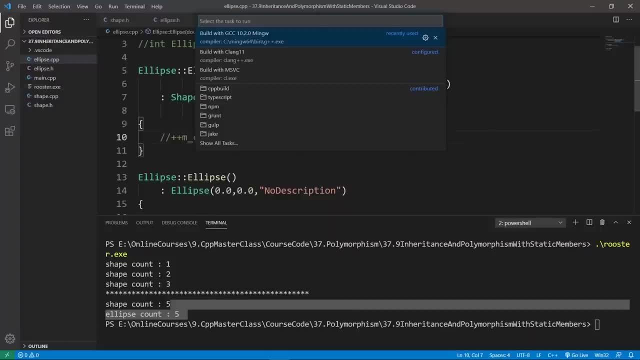 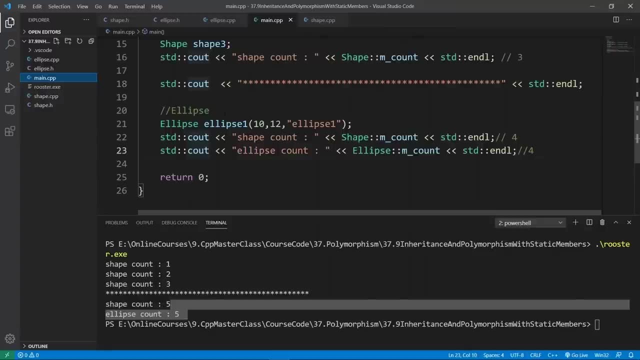 now we're going to build and really solve this problem. now you see the kinds of problems you can run into. if you have a static variable that is named exactly the same way and you have an inheritance hierarchy, really weird problems can pop up and you need to be aware of this. let's 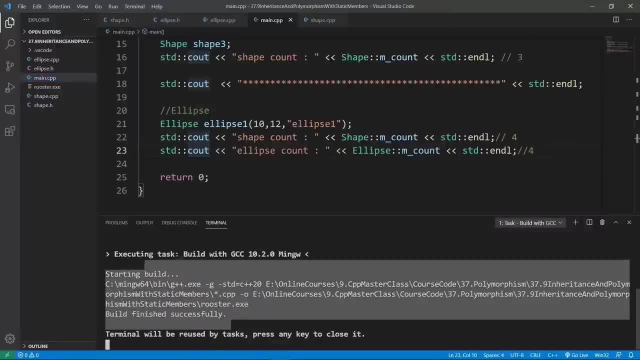 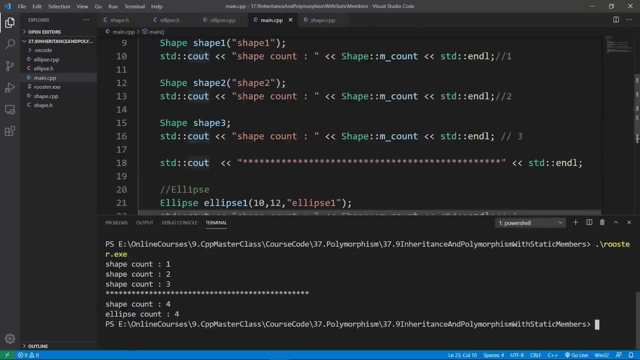 build and see that the problem actually disappeared. okay, the world is good. we can clear and run rooster. we're going to see that now. this is what we expect: one, two, three, because we have three shapes created up to this point here. if we create an ellipse, that's going to be another shape. 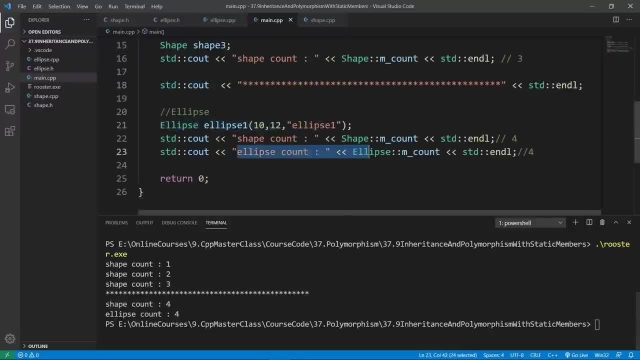 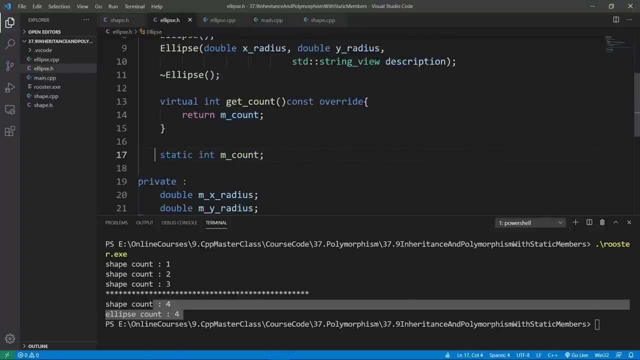 if we get the shape count we're going to get a four. but ellipse count is also giving us a four because ellipse doesn't have its own static variable. to solve this problem, we can go to ellipse and set up our own member variable at the ellipse level so we can enable this and uncomment it. we're going to go to the cpp file. 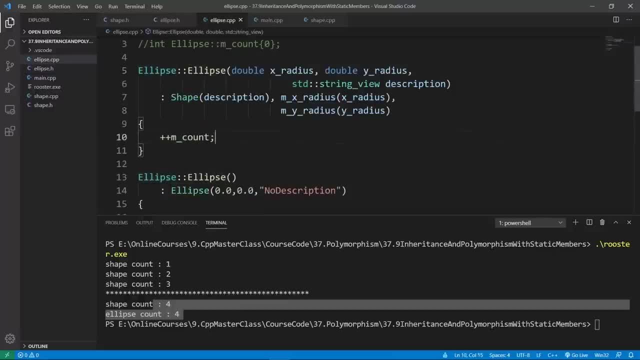 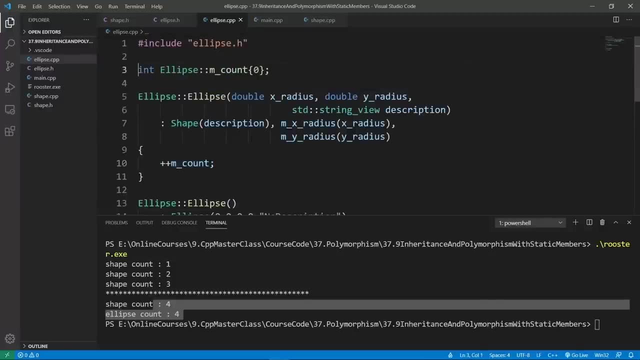 and make sure we are incrementing to get the correct count incremented here. i think this is all we need to do. we are also going to initialize the static variable we have at the ellipse level. this is going to do what we want and we can build again. now we're going to get the behavior we want. 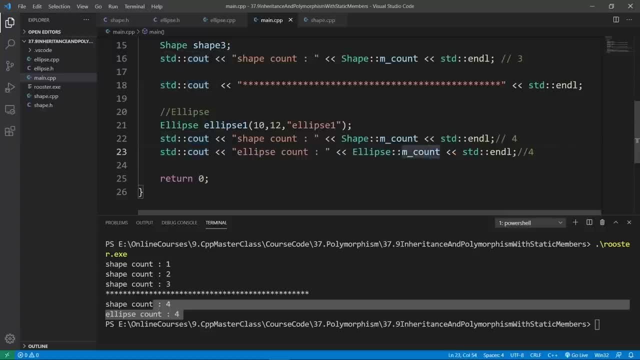 this point we are going to print a one for the ellipse count and this really makes sense because we have one ellipse even if we have four shapes in total. so this is the design i think makes more sense in our c plus plus program. here we are going to build this again and pass this through gcc. 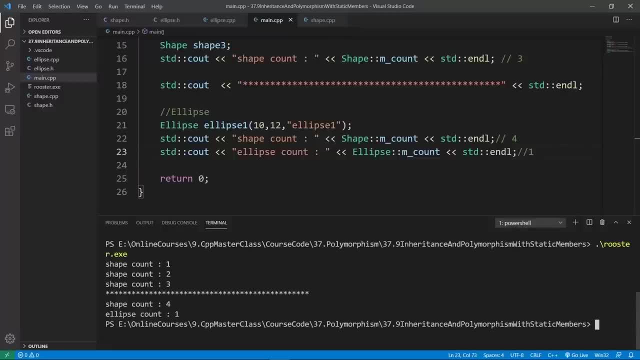 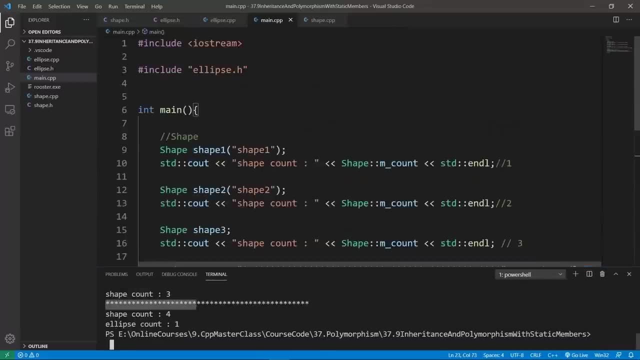 the build is going to be good. we can clear and run rooster. now we're going to see that we have four shapes and one ellipse, and this is what we want. now that we have this, we're going to continue to print the shape count so we can really do all kinds of crazy things, hopefully. 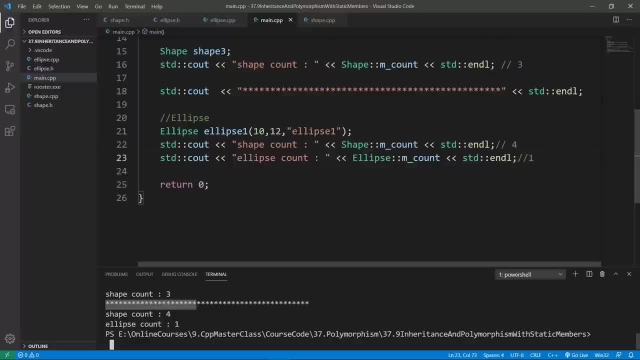 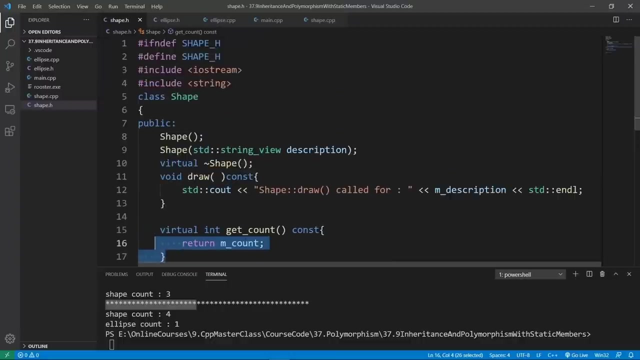 you can see that the static variable is working exactly as we want. we can print the ellipse count, we can print the shape count if that's what we want in our c plus plus program. but we can also do shape polymorphism and get the correct get count method called in our c plus plus program. 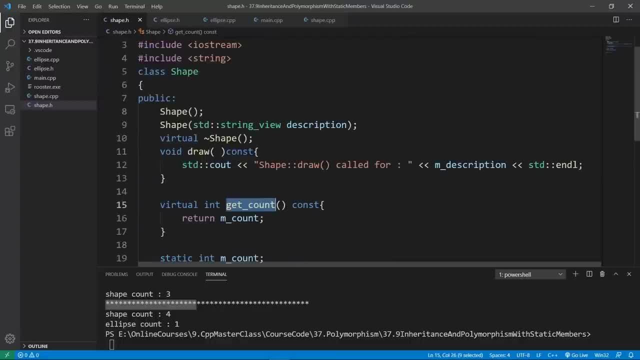 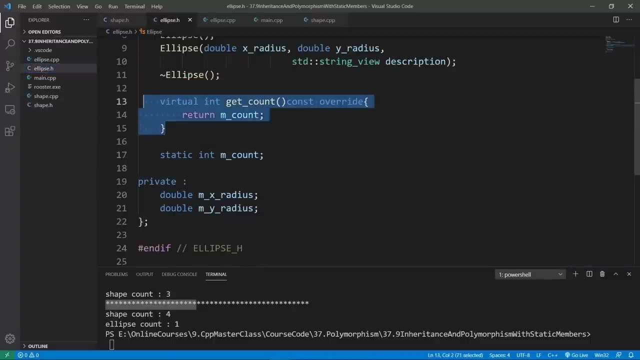 for example, if we call the get count method on a base pointer, that is managing a shape. we're going. that is managing an ellipse. we're going to get this one called. this is going to be super cool. let's go up in our program and set this up. we're going to do this on the fly. let's say shape. 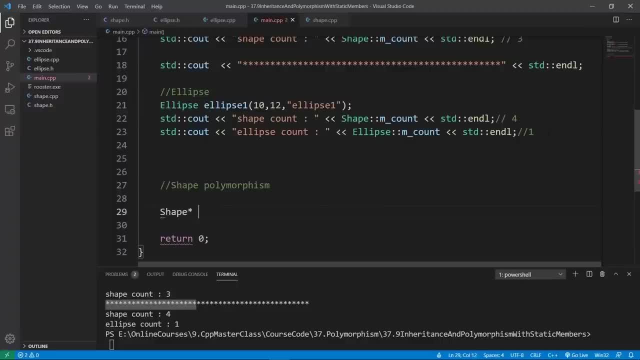 polymorphism, and we're going to say shape pointer, and it is going to be an array. let's say shapes, this is going to do and it is going to be just an array, and we're going to initialize this and store in a bunch of objects. let's put in our closing brace here. let's go up and see what we 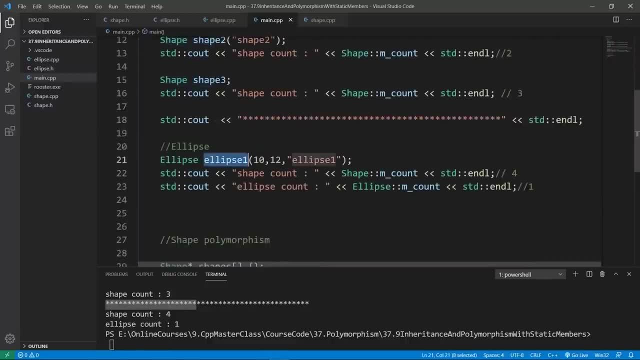 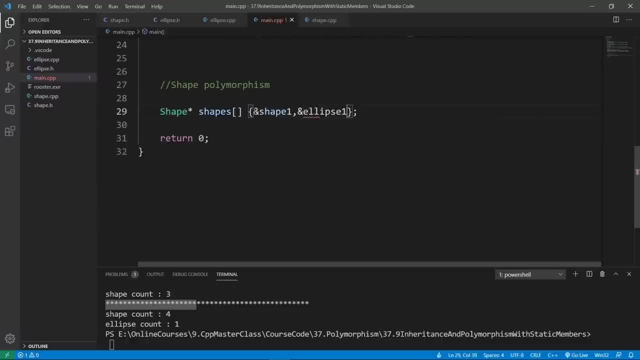 have. for example, we have shape one and ellipse one. we can use these. we're going to put in the address of shape one and we're going to put in the address of ellipse one. this is going to do and we can loop through these guys and call the get count method. so let's do this. we're going to. 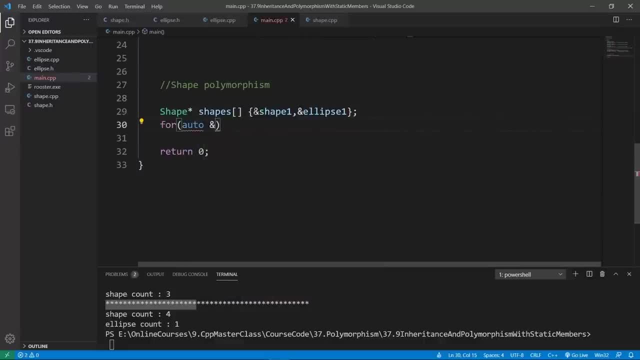 say for auto s and let's do a reference because we don't want copies, and we're going to say in shapes and we're going to call the get count method. we're going to say s and say get count. this is going to give us the count and we can print this out if we want. we can say sddc out and count and we're going to. 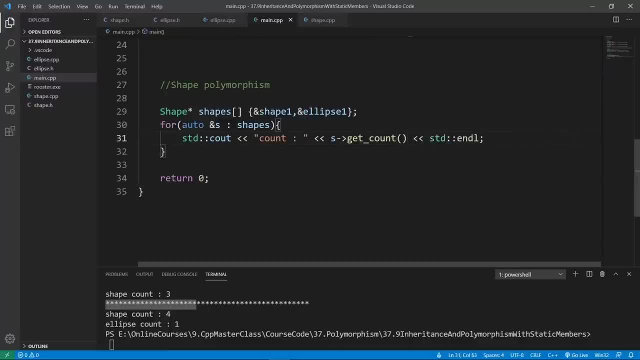 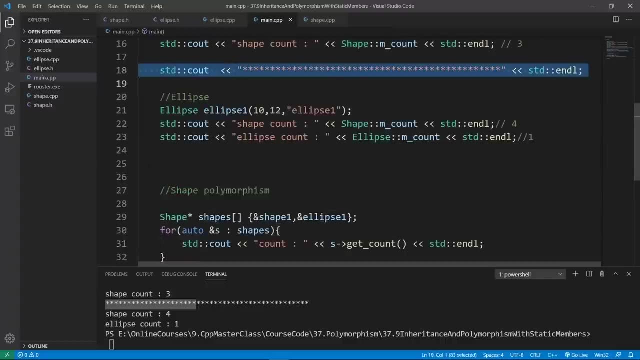 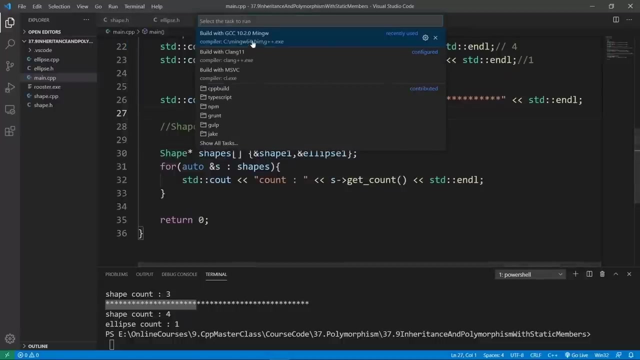 put a new line character here to separate these guys, and we can put a separator here. we can copy what we just used in our c plus plus program here, just to make sure this is super clear when we print things on the terminal here. we're going to build our program and see if it actually works. 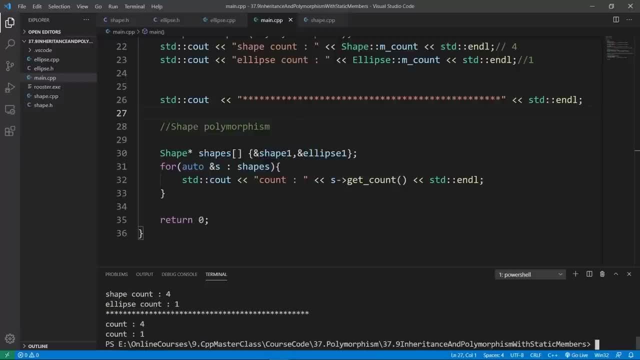 the build is going to be good. we can clear and run rooster. we're going to see that the count is going to be four for the first iteration because we're going to be calling the get count method from shape, because that's our base pointer. so this is what we're going to get. 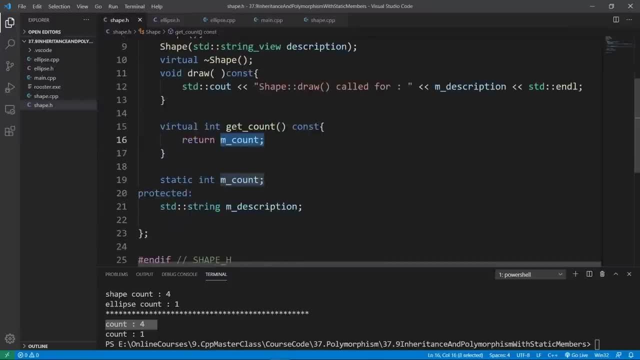 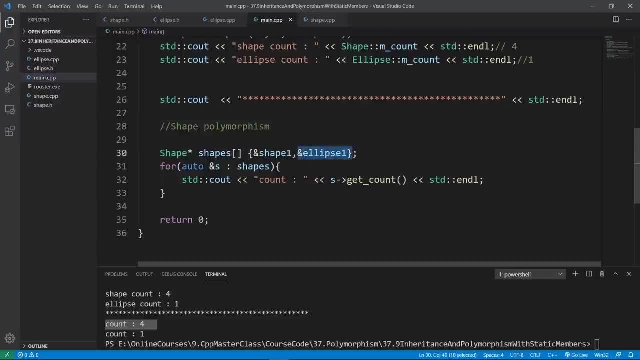 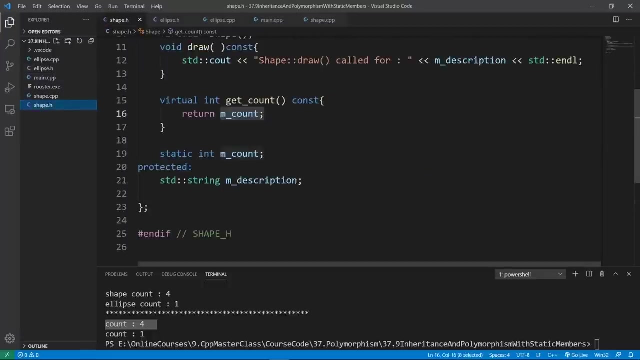 we're going to print the m count member variable from the base class. that's why we have a four. but on the second iteration the object is ellipse and we are using polymorphism because we are going through a base pointer and this base pointer happens to support the virtual method get count. 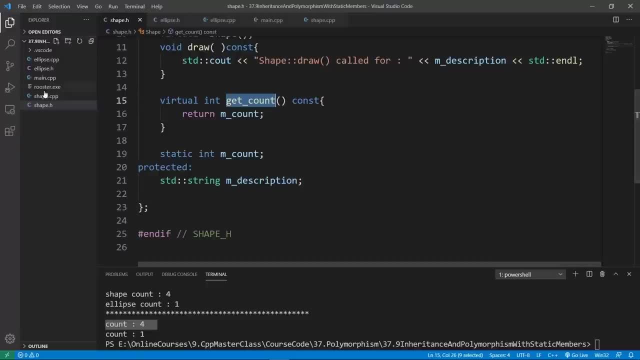 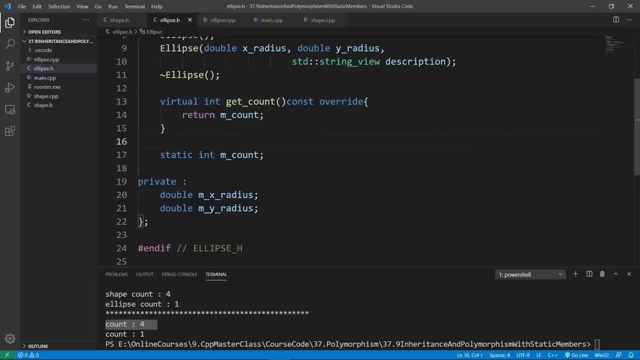 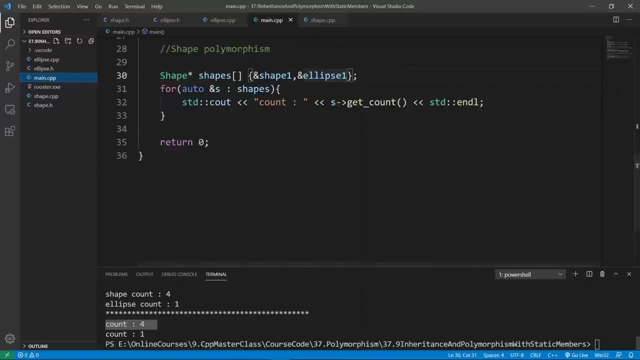 we will get the most specific one, called on the current object that our base pointer is managing here, and this happens to be an ellipse. so we're going to call the ellipse version of our virtual function here and we will get a one, because we really have one ellipse in our c plus plus program. 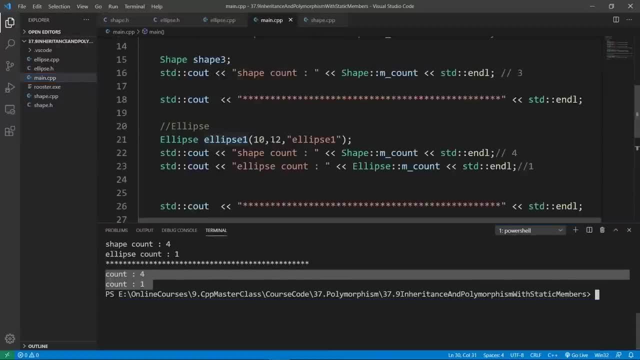 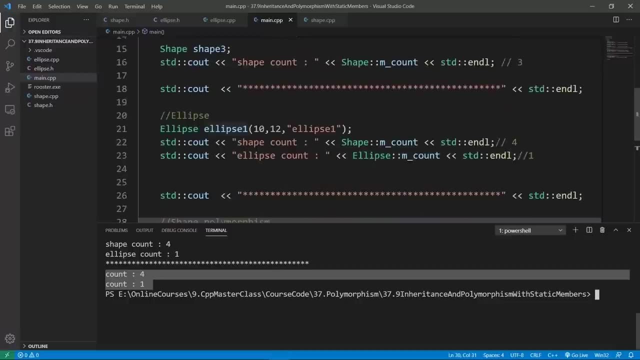 this is what we see here. this is really all i wanted you to see in this lecture: how you can use static member variables with inheritance and polymorphism, and you need to be aware of these little things that are going to be used in this lecture. so let's get started, and let's get started. 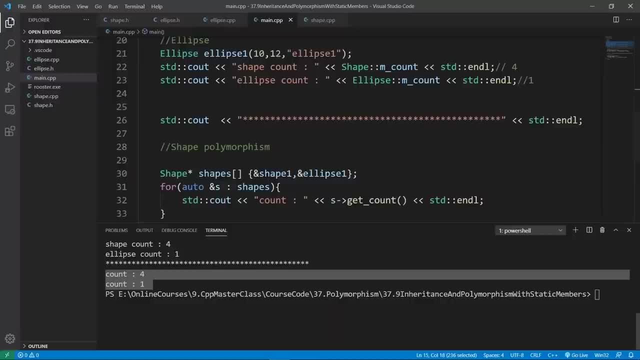 that can really be confusing, especially for beginners. we are going to stop here in this lecture. in the next one we're going to learn about the final specification we can use in our inheritance hierarchy. go ahead and finish up here and meet me there. go ahead and finish. 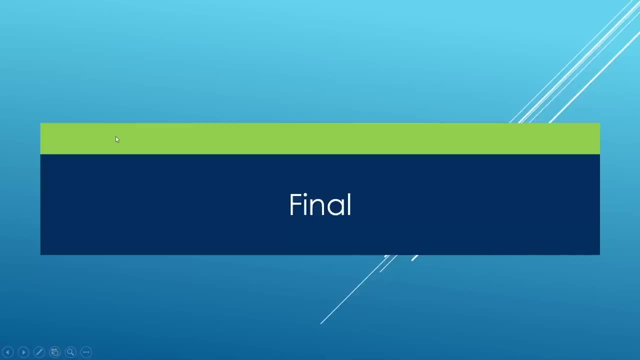 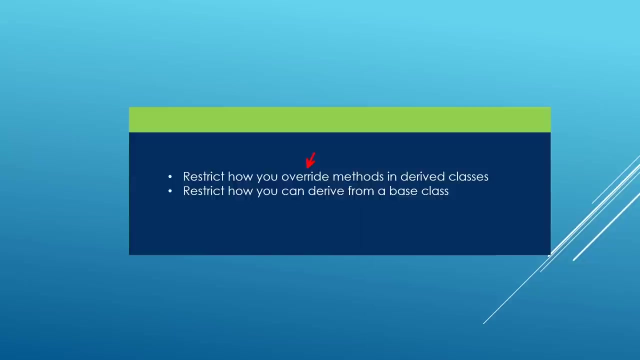 up here and meet me there. in this lecture, we're going to learn about the final specifier used in inheritance hierarchies. this is going to allow you to do one of two things: you will either be able to restrict how you override methods in derived classes, or you can restrict. 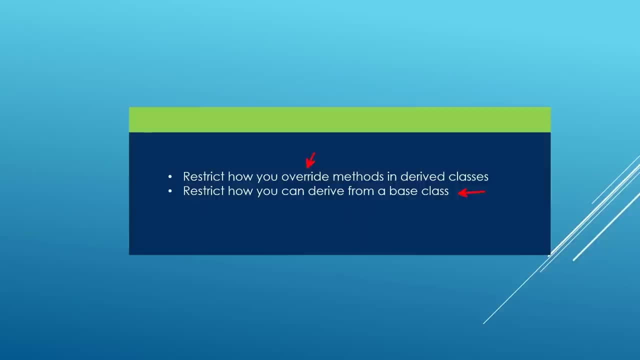 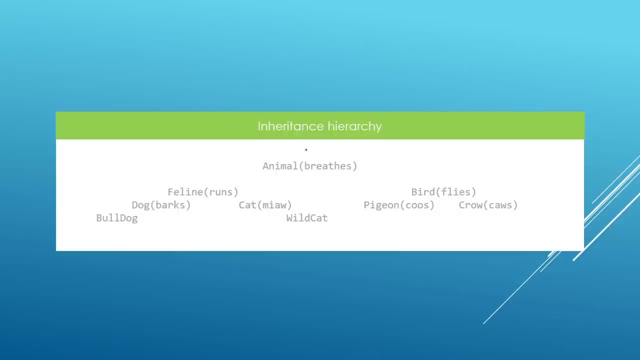 how you can derive from base classes. i know this is in the air, but we're going to look at a few examples to really drive this home. suppose we have an inheritance hierarchy like we see here. the top class is animal. we can derive from this and have feline. you can have bird as a derived class feline. 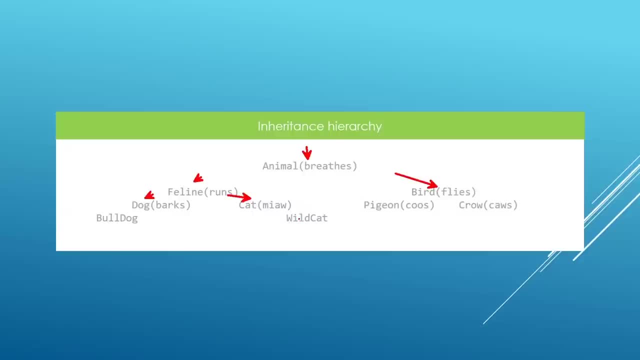 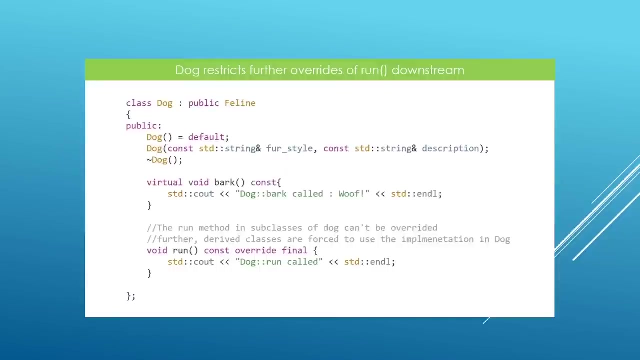 can be inherited to have a dog and cat, and you can derive from cat, for example, to have wild cat, and dog from dog. you can do all these things here, and this is inheritance hierarchy we're going to be using to learn about these things now. here is a possible implementation for the dog class, which 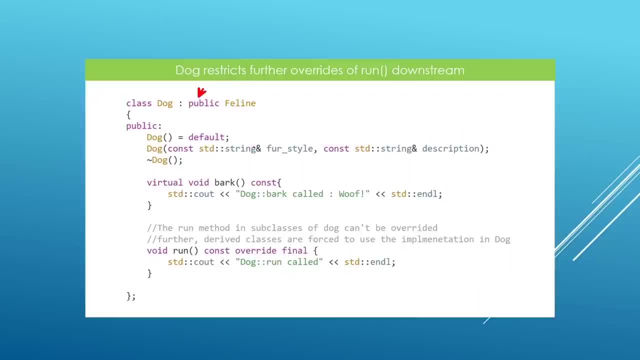 is going to be inherited from feline publicly, as we see here. but take a look at the run method we are setting up in dog. we are appending a final specifier and what this is going to mean is that no downstream inheritance class will be able to override. 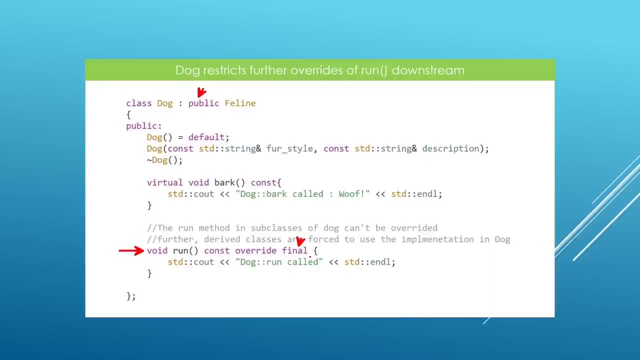 the right method. further, this is what we can achieve. so if we don't want our derived classes to override our virtual method, we can mark that method as final in our class and we are basically saying i am going to put in my implementation, but i don't want any deriving downstream class to 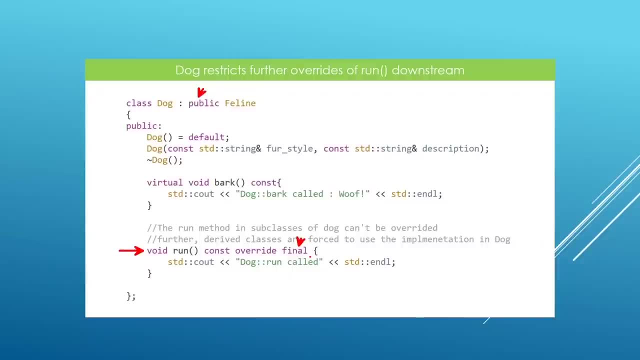 override this method further. if they do that, they are going to get a compiler error, and this is something we can achieve using the final specifier in our inheritance hierarchy. again, in this case, we are using this to restrict how people can override our own virtual method in downstream classes, or i shouldn't really say our own method, because 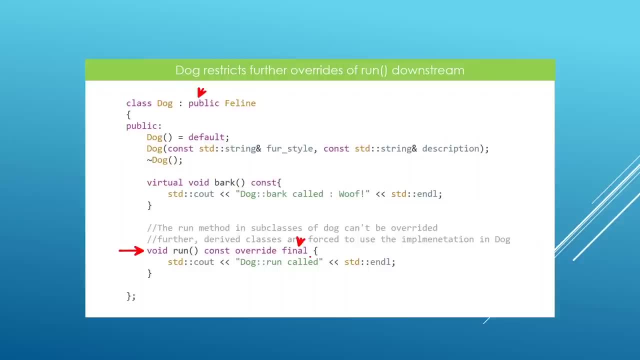 it may be coming from upstream, but you are restricting people from overriding that method further in downstream classes here. okay, so this is the first use we have for the final specifier, but we can also restrict people further in the downstream class. the v Arduino커 계산 �ue Нетjedка kmkIMk race. may be that we are now overriding people, so it is thus one way to유를ž Tub desde birdie considerably further up, ps. 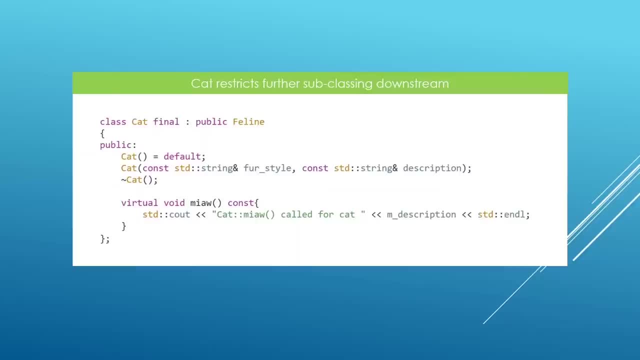 from inheriting altogether. so here we have a simple example to drive this home. we have our cat class. it is going to be inheriting from feline, but we are marking our cat class as final and what this is going to mean. if anybody tries to inherit or derive from cat in any way, they are going to 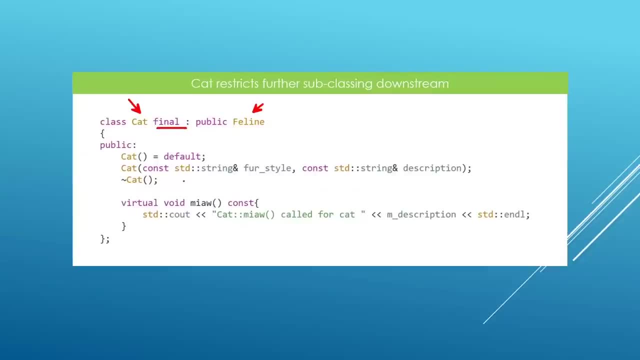 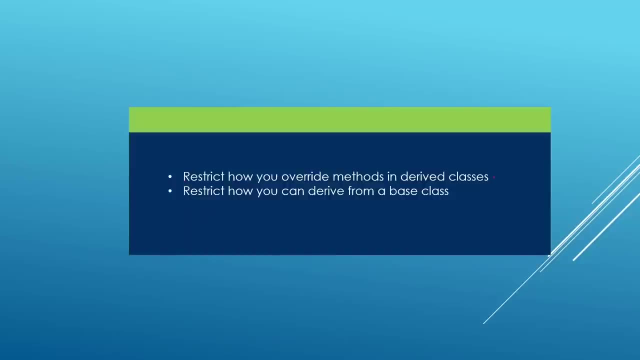 get a compiler error, and this is what we can achieve with the final specifier. again, there are two things. you can restrict how people override your virtual methods. if you want to restrict that from the current class, you can mark your virtual method as final. you can also restrict. 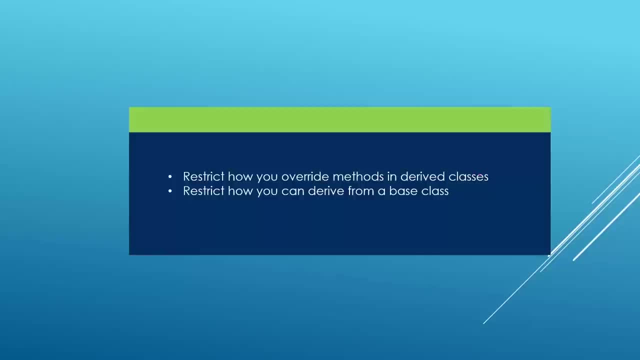 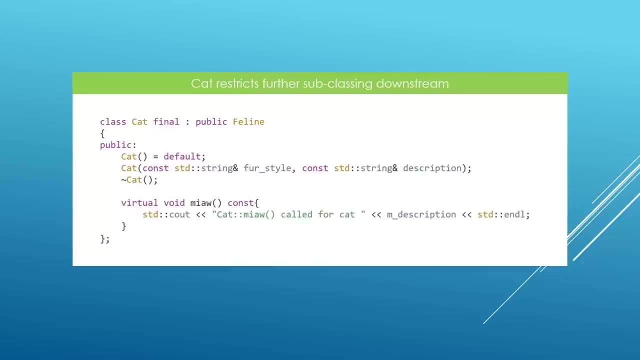 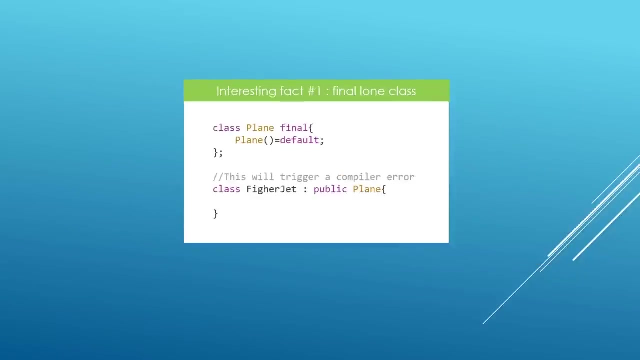 how people inherit all together from your class, and if you want that behavior, you can mark your class as final using the syntax which are so in the slides here. okay, now that you know these things, let's look at a few things that may be interesting. for example, here is a simple fact that you can 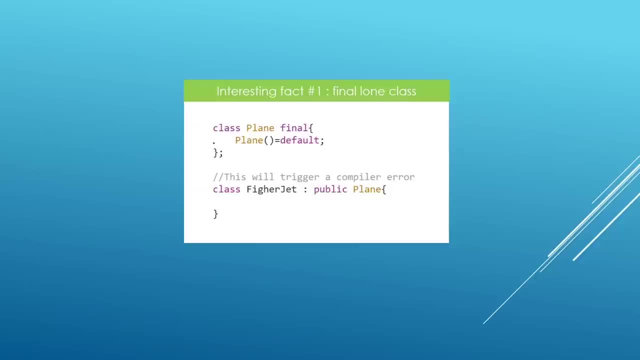 create a class right away and mark it as final, and when you do this, nobody will be able to ever inherit from this class in your program, and if we do this, we will get a compiler error, for example. this is one thing i find interesting and i really wanted you to know this. another thing: 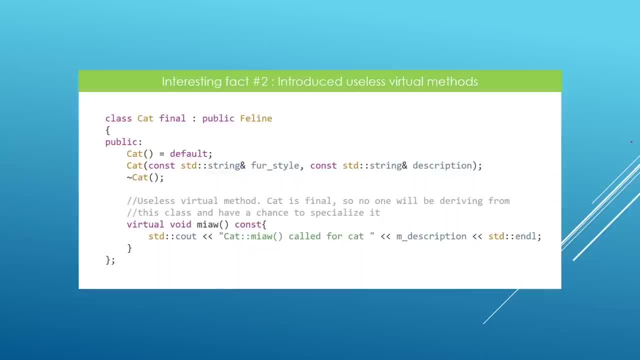 is that it is possible to introduce useless virtual methods in your inheritance hierarchy. for example, if our cat class is marked as final, what this means is that nobody will ever be able to inherit from this class. but we are going further and setting up a virtual method which is meant to be inherited or overridden in downstream classes. but how do we get to? 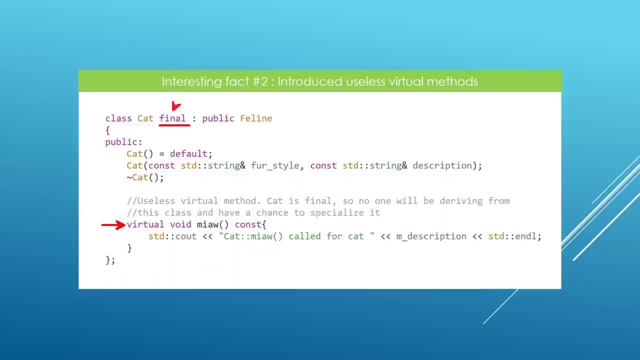 downstream class if we can't inherit from the cat class, which is marked final. so so we have conflicting ideas here. on one hand we are saying we can never inherit from this cat class, but on the other hand we are setting up a method that is meant to be used or specialized in a derived 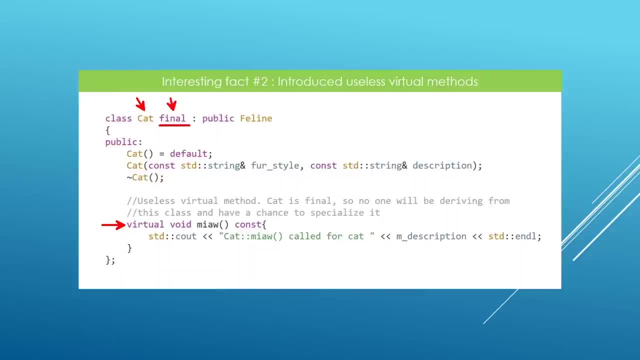 classes. so this is something that is interesting. this code is going to compile and i think maybe in future standards of c plus plus they are going to fix this problem and maybe give you a compiler error if you try to do something like this, but at this point you're not going to get a compiler error. 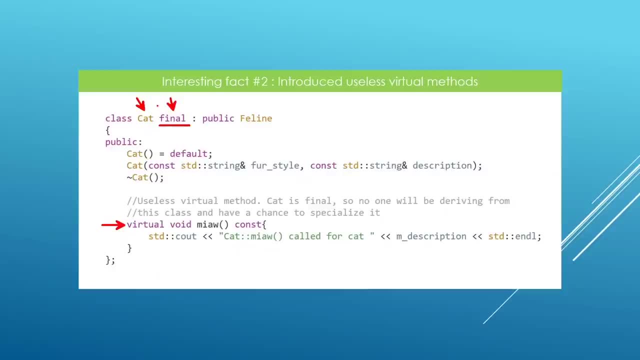 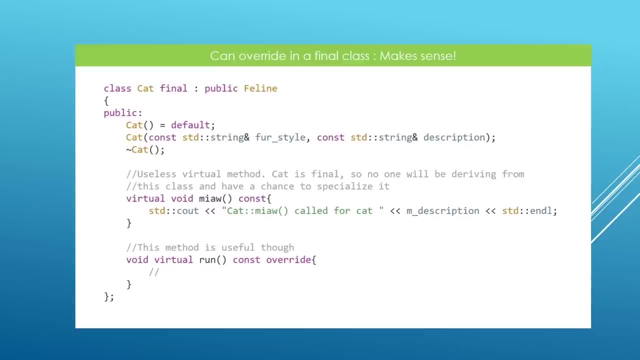 this is just going to be valid c plus plus syntax. even if this is really weird, we have conflicting ideas here, okay. one thing you should know, though, is that we can override in a final class, and this is going to make sense because, for example, the run method is coming from the feline class, and here we are just specializing that, so we are. 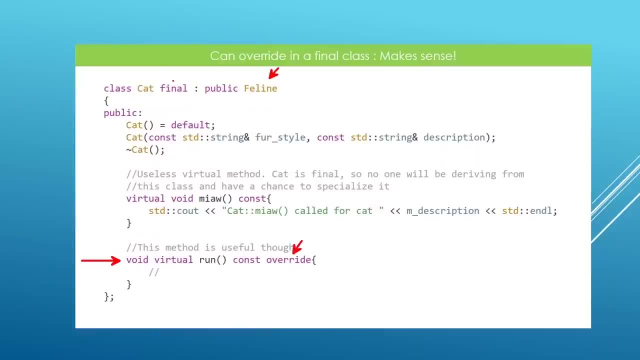 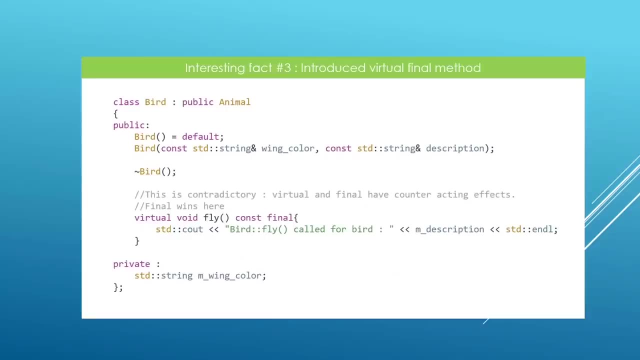 marking that as an override here, even if this is a final class. so be careful: this is valid c plus plus syntax. this is going to work just fine. another thing you can do, which is pretty useless in your c plus plus program, is to introduce a virtual method and mark it as final right away. so again, 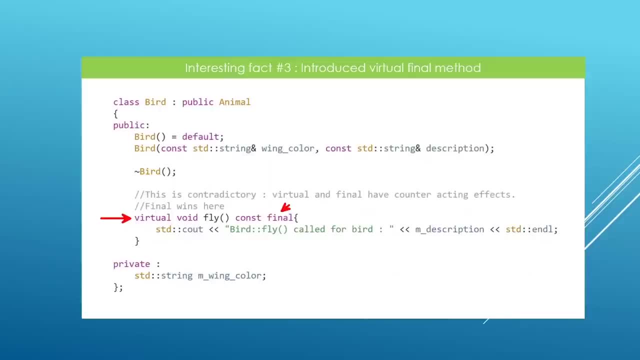 this is really weird. we have two i ideas that are conflicting. the virtual keyword means that we want this to be specialized in the downstream classes, but again we are saying: this method is final, so no downstream class will override this. if they try to do that, they are going to get a compiler error. so this is again. 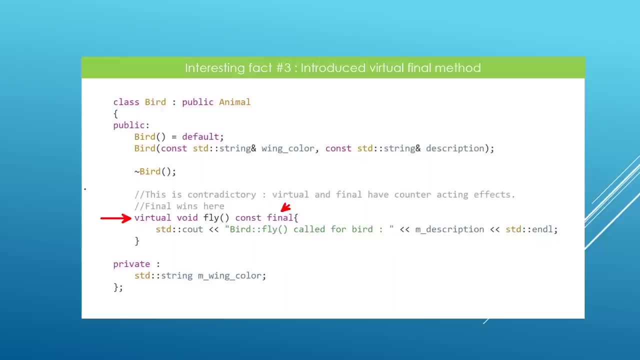 a bunch of conflicting ideas. c plus plus is going to allow this syntax. this is not going to give you a compiler error, but this is weird and you need to be aware of this. okay, now that you know these ideas, we're going to head over to visual. 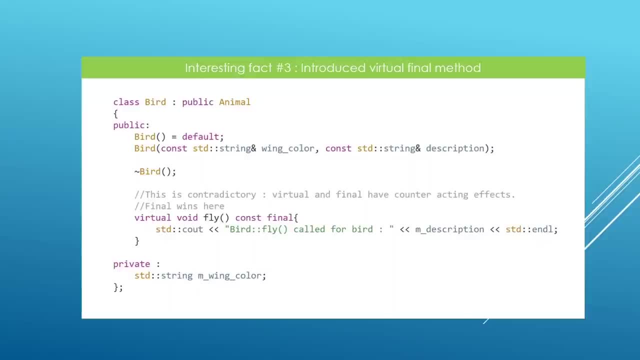 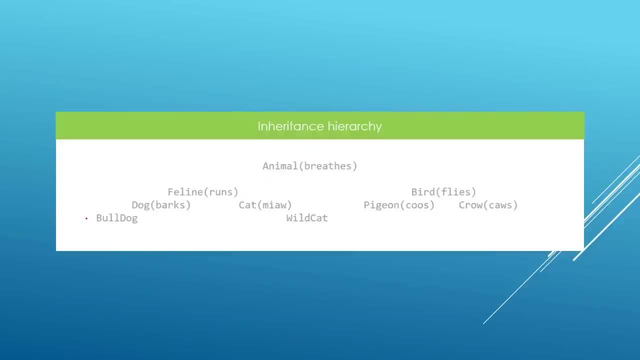 you know these ideas. we're going to head over to visual. you know these ideas. we're going to head over to visual studio code and play with the final specifier in our inheritance hierarchy. we will be setting up this kind of inheritance hierarchy and we will set up a bunch of virtual methods and mark them as. 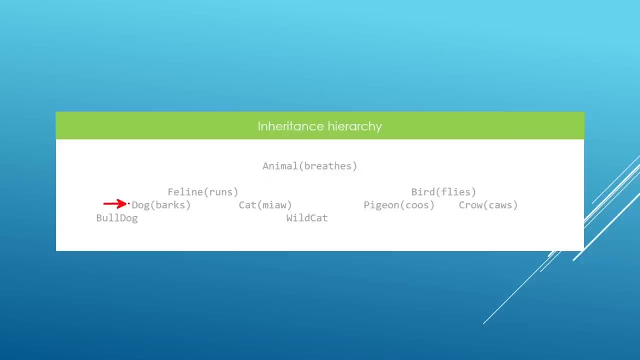 final. i think we will do that in the dog class and we will mark a bunch of classes as final and see that if we inherit from them we're going to get a bunch of compiler errors. so let's do this. here we are in our working folder. the current project is final and 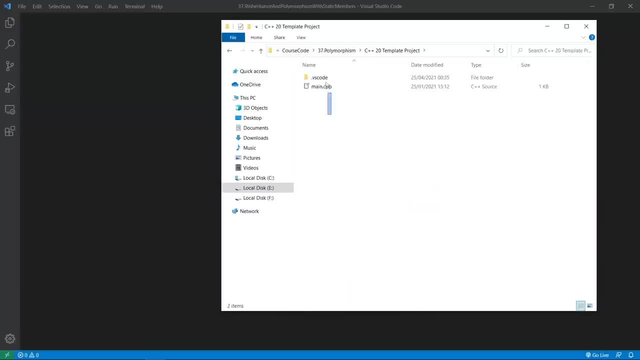 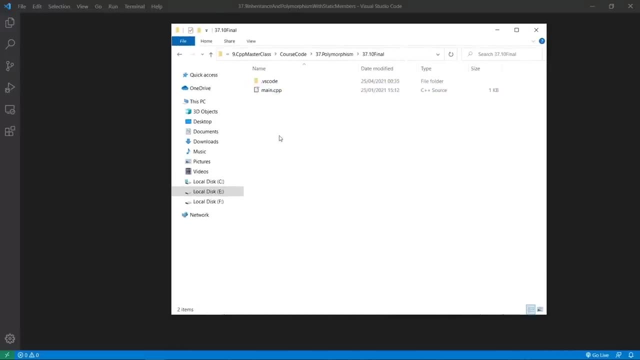 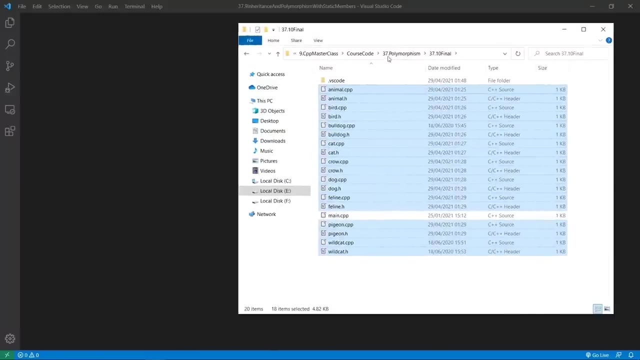 we are going to bring in our template files pretty quick. we're going to use this as our starting point. we're going to put that in place and i am going to put in a bunch of classes i have lying around on my system because i don't want to set up these classes. that would be a waste of your. 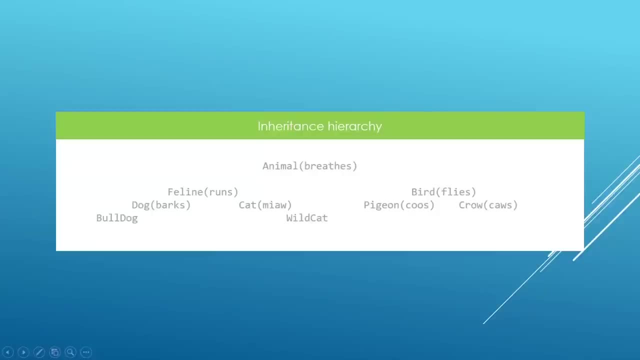 time. just know that we are trying to set up this kind of inheritance hierarchy: animal is going to be our top dog or animal is going to be our top class, and we will be inheriting from this, creating an inheritance hierarchy. and we will be inheriting from this, creating an inheritance hierarchy, and we 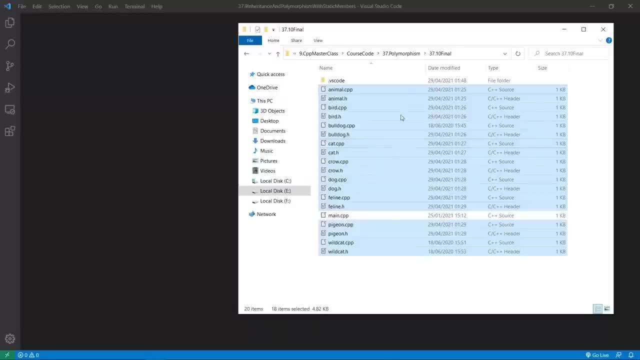 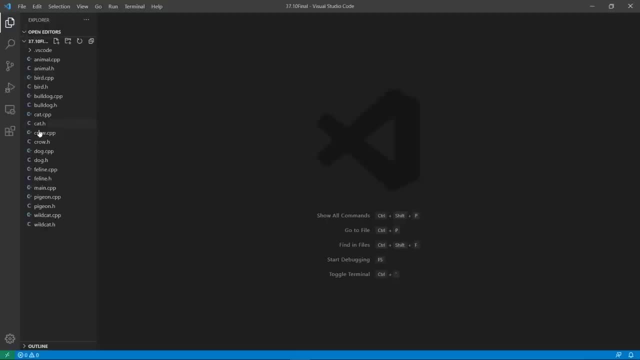 inheritance hierarchy we can play with in our code here. okay, so we are going to open this up in Visual Studio code, so let's do that by dragging and dropping here. this is going to give us all these crazy classes we have. the top class is going to be animal and it is going to be defining the. 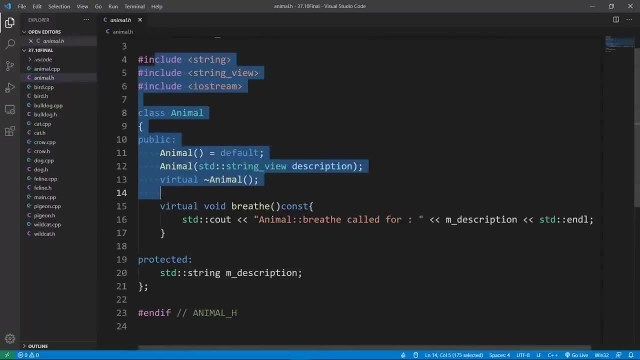 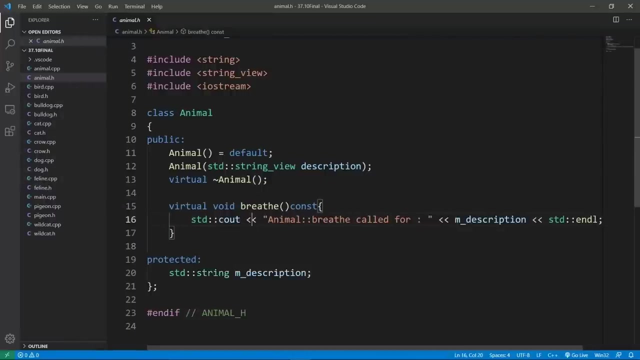 features any kind of animal with support in our C++ program is going to have. for example, any kind of animal will need to breathe and we will set up this virtual method here and we will be inheriting from this animal class to create a feline class and a bird class. this is something we did in a 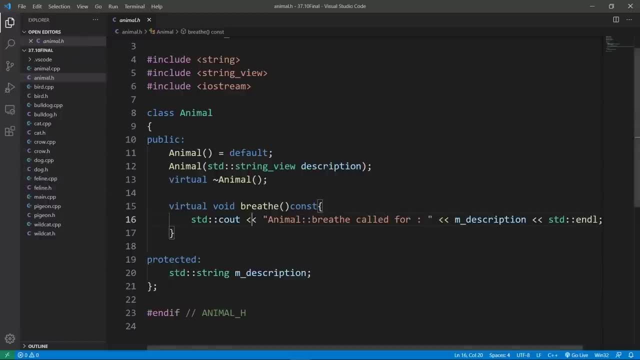 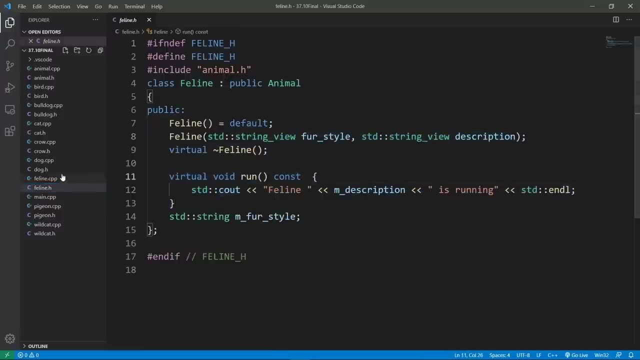 few previous lectures and we are just reusing this inheritance hierarchy here. let's look at the feline class. the feline class is going to set up a virtual method which is called run, and the method is going to be overridden. in the dog, for example, we can override the run method, but 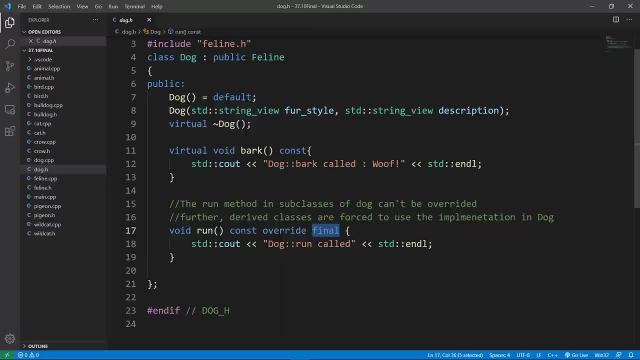 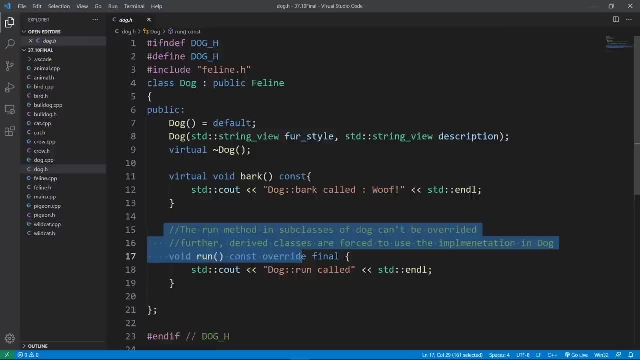 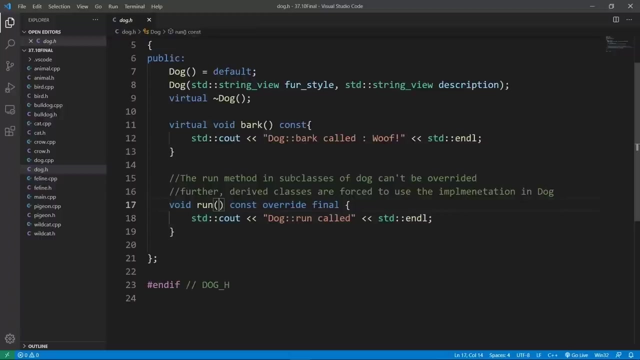 notice that we are marking that as final. okay, so look at this: the method is final, and what this means is that no downstream classes inheriting from Doug will ever be able to specialize or override this method further. if they try to do that, they will get a compiler error. 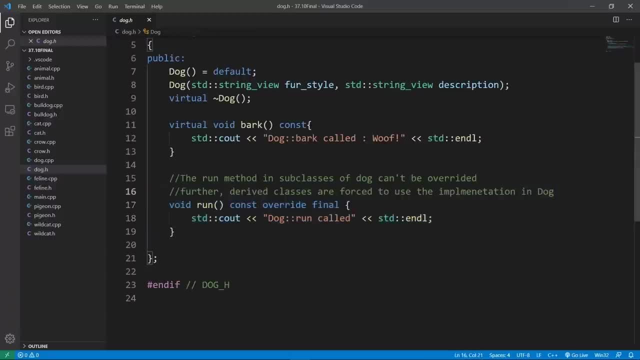 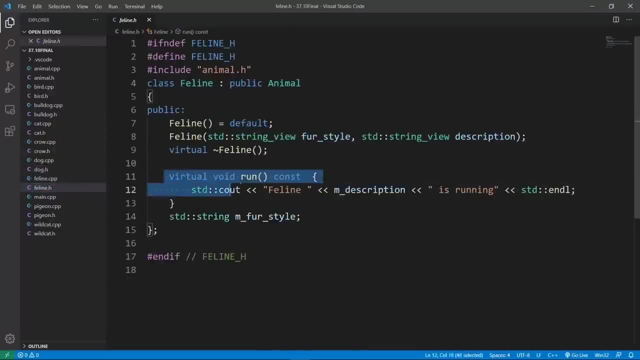 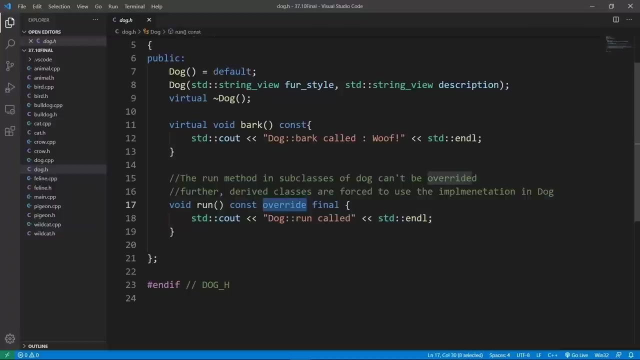 notice that this may be our method or it may be a method coming from upstream classes. in this case, the run method was introduced at the feline level. you see, it was introduced here and Doug happens to be overriding this method here. that's why we have the override keyword, but at the same time we are going to mark it as final and prohibit, or 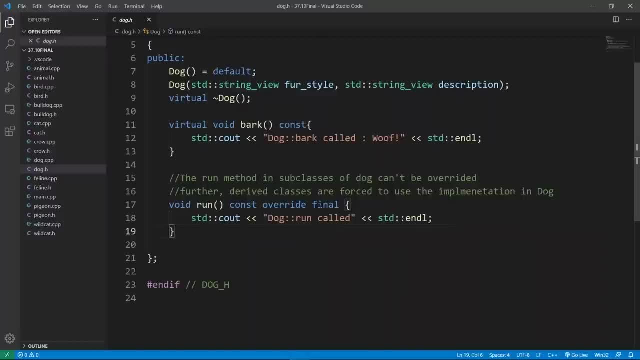 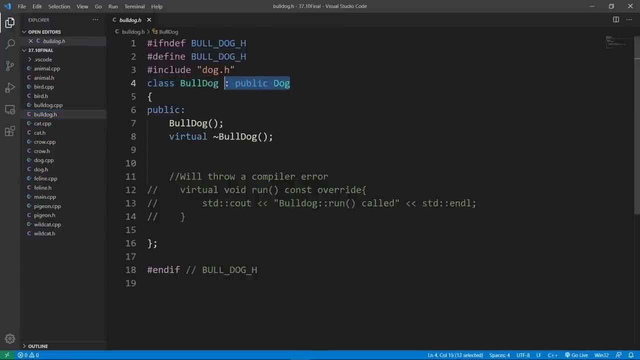 prevent downstream classes from overriding this method. further, if we look at our Bulldog class, we're going to find the class to inherit from Doug. we have our run method here. it is commented out at this moment. I just want you to see that our code is just going to compile. if we compile it now, let's. 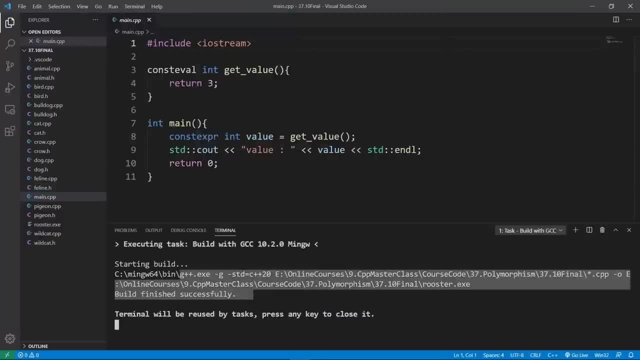 go, we're going to pass this through GCC, okay, you see, the build is good and we have generated our binary, which is really not doing anything because our main function is just some dummy code we have here to make sure it works with C++ 20, but what I want you to see is that if you go in Bulldog, let's. 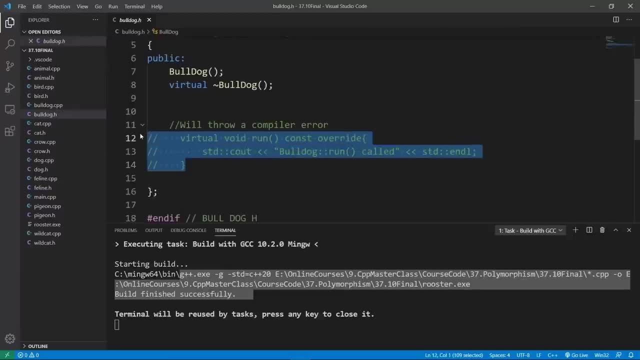 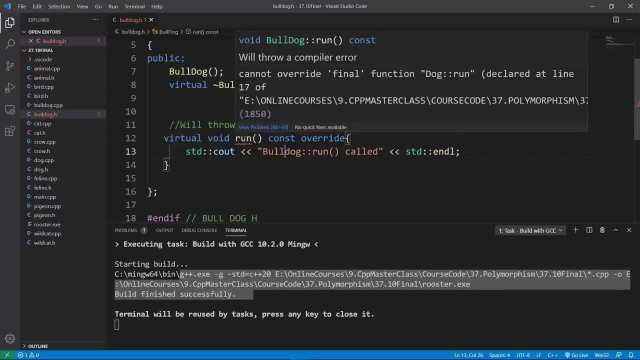 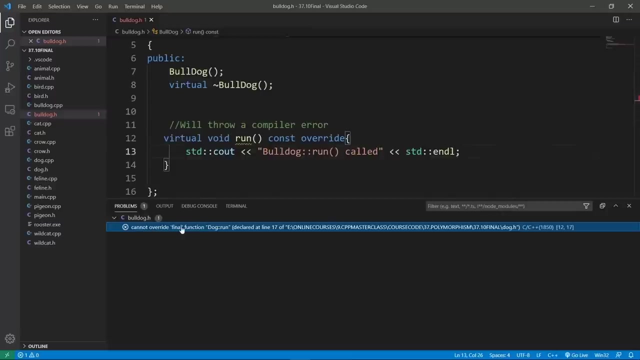 go in our Bulldog class and uncomment this class here or this virtual method, we're going to see that we're going to get a compiler error. we have a squiggly line meaning that we did something wrong and we let's look at the problems. tab from Visual Studio code here cannot override final function. 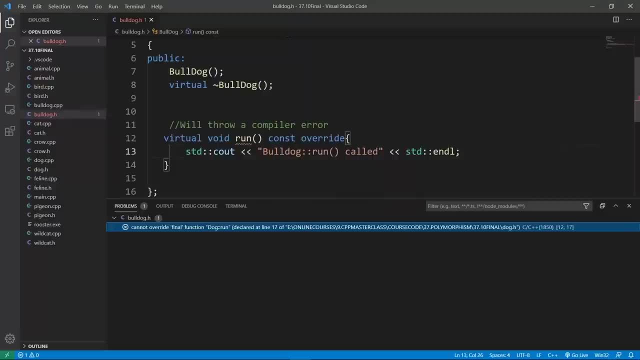 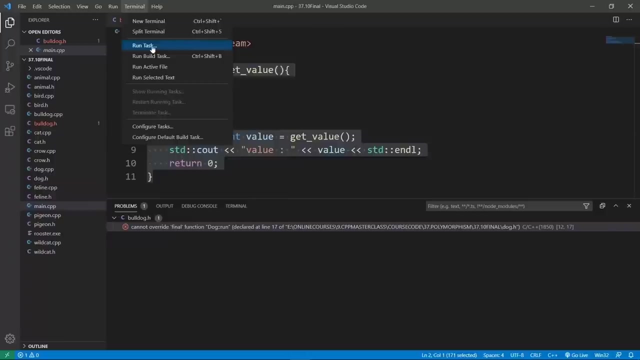 Doug run. this is a final method from the dog class. if we try to override it further, we will get a compiler error. this is something we can achieve by marking our virtual method as final, as we are doing here now. if we try to build this program, we're going to get a compiler error. let's pass this. 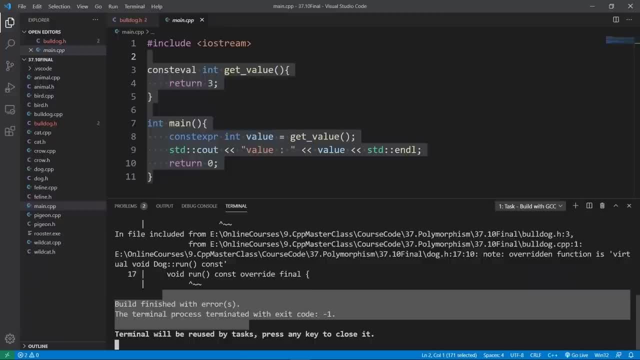 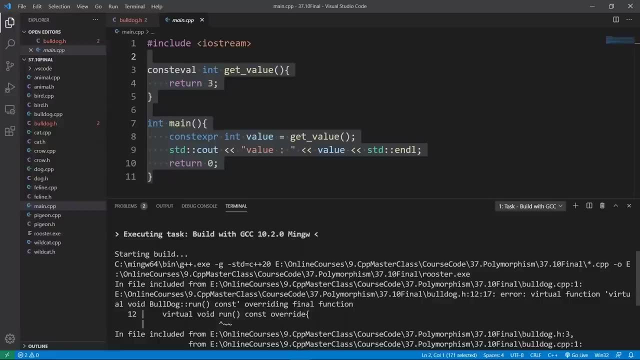 okay, you see we get a compiler error and, uh, the error is that we are overriding. let's go up and see the error here. error. and on line 12 in Bulldog H we see that we are overriding a final method, virtual void. Bulldog is a final function and we are overriding this and this is going to give us. 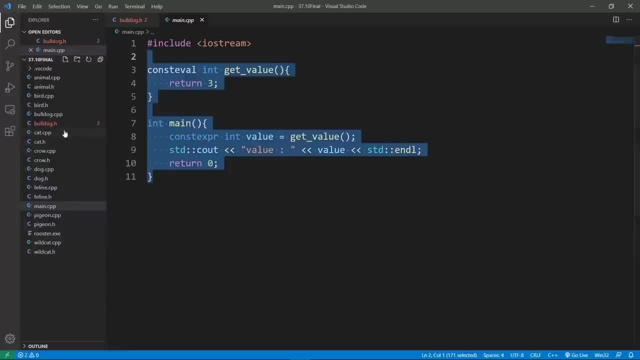 a compiler error. this is the behavior we get. so the message here is that you can go in your inheritance antenna level and mark a virtual method as final and prevent downstream classes from specializing or overriding that method further, and if they do that they will get a compiler error. this is 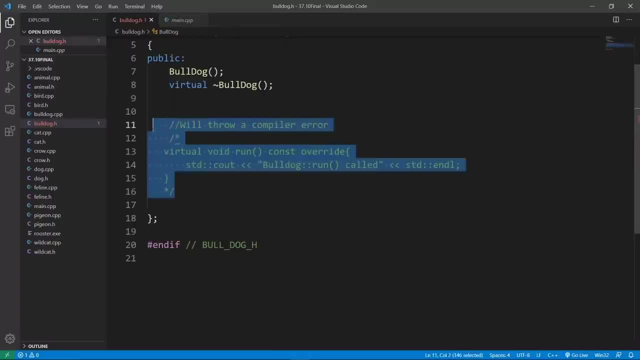 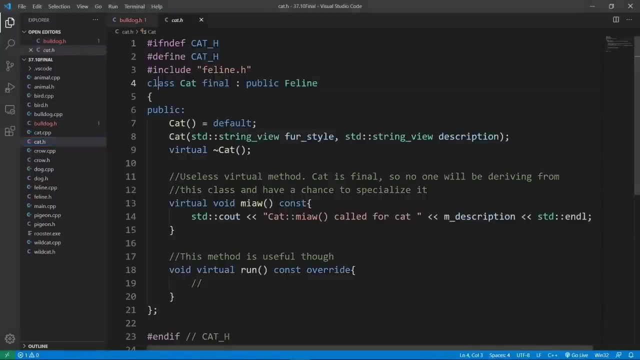 something we can achieve in our c++ program. another thing you can do with the final specifier is that you can prevent people from inheriting from your class altogether. let's go to our cat class. I think that's the example that sets that up. we have a cat class. it is going to be inheriting from feline, but the class is marked as final now. 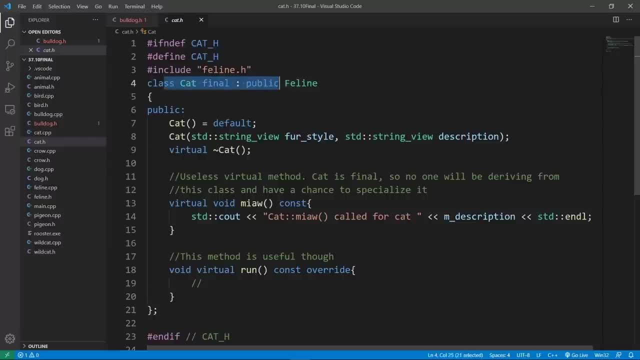 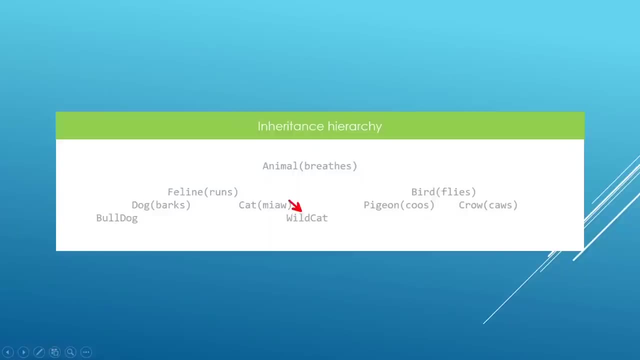 what this is going to do. it's going to throw a compiler error anytime somebody tries to derive or inherit from this class here. so if somebody tries to inherit from cat, as we are doing here, create a wild cat from a cat, we are going to get a compiler error because we can't inherit. 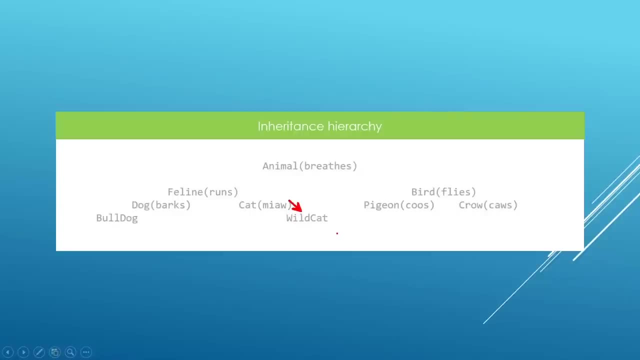 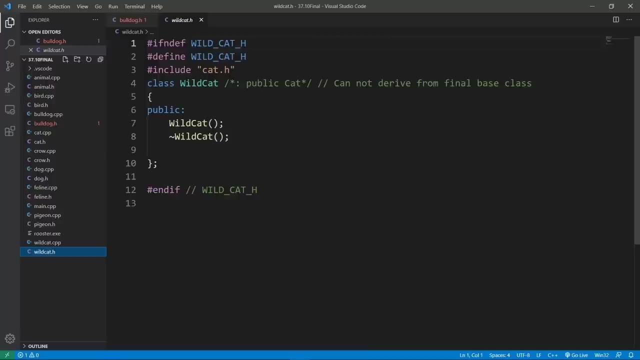 from cat altogether. it is a final class at this moment. okay, so let's look at our wild cat class. it is going to try and derive from cat. we can do something like this. we can remove our comments here, and if we're trying to do this, we will get a compiler error. let's look. 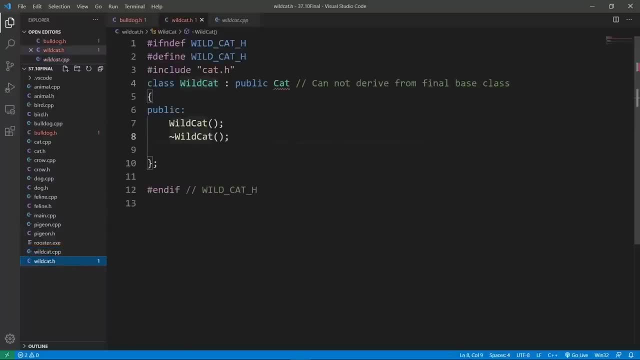 at the cpp file and see what we have. it has nothing special, but if we try to do that and inherit from cat, we will get a compiler error because the cat class is final and you cannot derive from it. if you do that, you will get a compiler error because the cat class 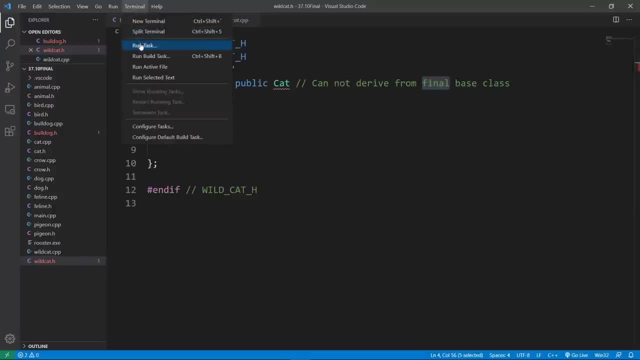 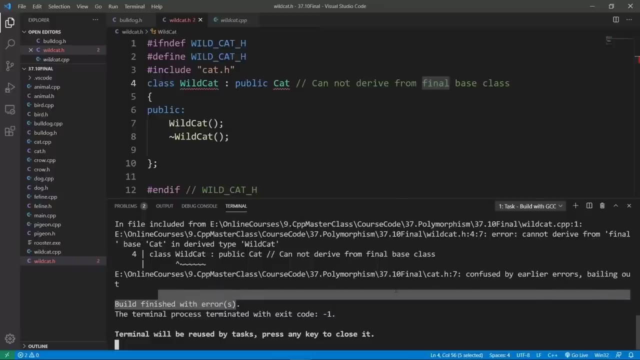 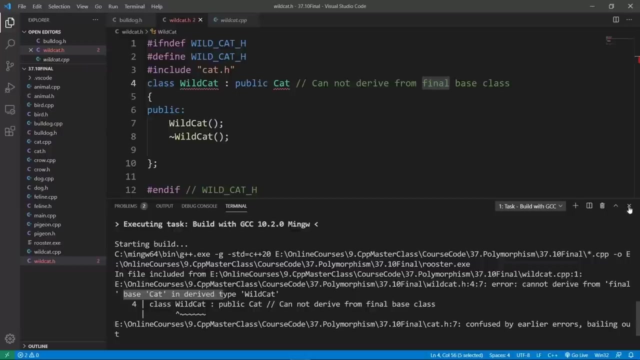 is final. this is what I want you to see here. let's try and build our program again. we're going to pass this through gcc and we will see our compiler error. okay, the world is finished with errors. if we go up, we will see that we cannot derive from a final base class. if we do that, we 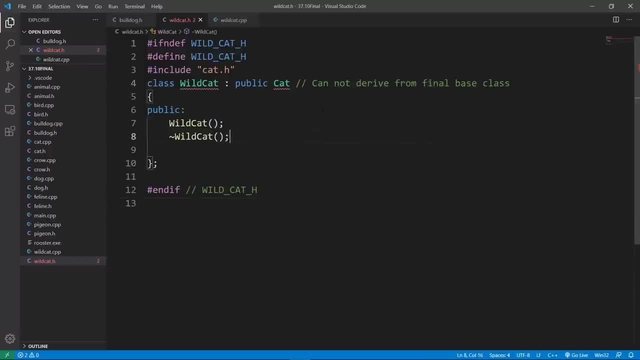 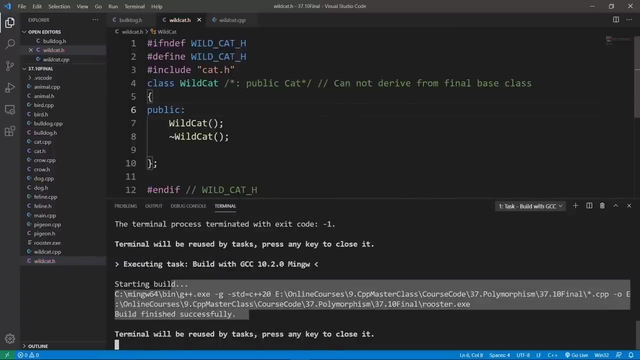 will get a compiler error, and this is what I want you to see here. okay, now that we know this, we're going to take this back and take out the compiler error here, because we want our code to compile. it is compiling, fine. okay, now the code is compiling because we are no longer trying to inherit from. 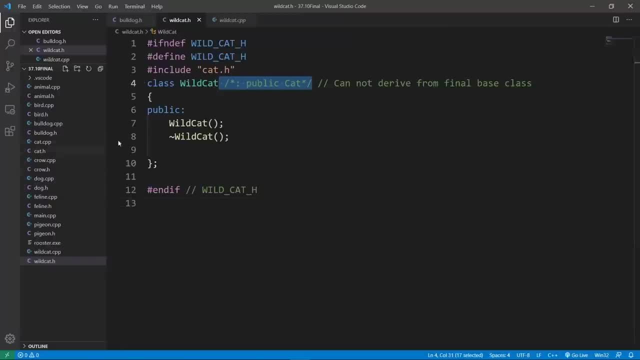 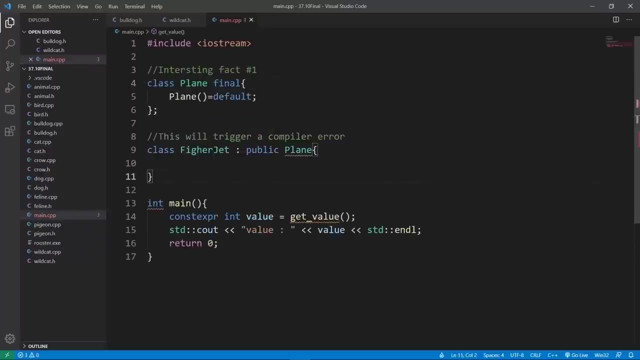 cat and I want you to now see a few interesting thoughts about the final specifier when it works together with virtual functions. let's go to the main cpp file and show you the first fact, and that's that you can create a class right away and mark that as vinyl as you create it, as we. 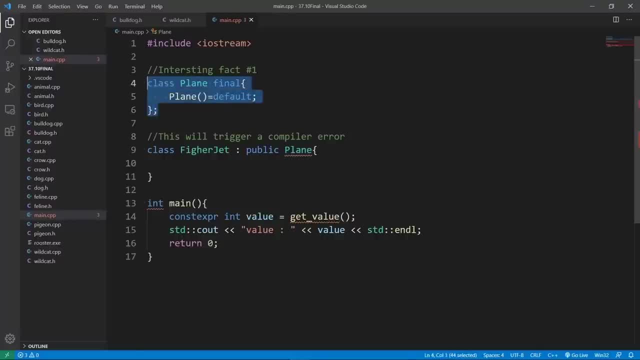 do here? if you do that, this class is going to not be inheritable, and if you're trying to inherit from it, you will get a compiler error. let's take out everything we have here and just say hello. in our main function this is going to do just to have. 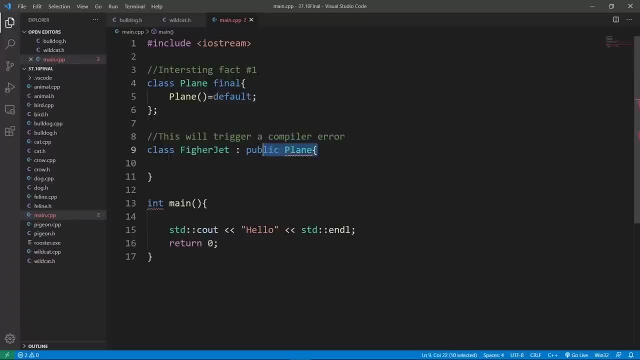 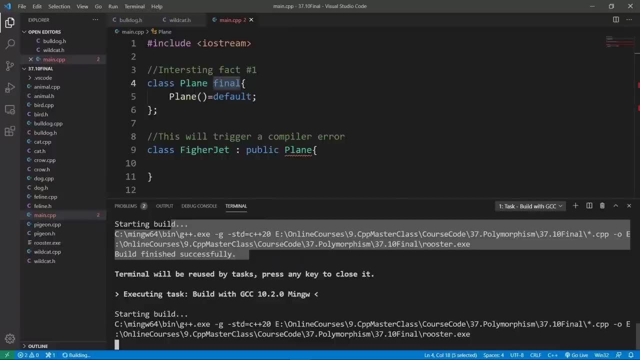 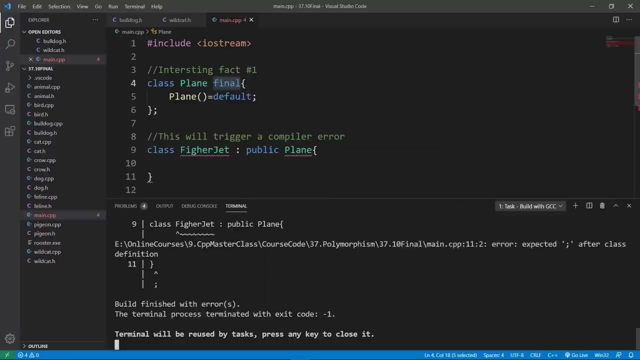 something. this is going to give us a compiler error because we can't inherit from a final class. let's build and show you the compiler error. this is going to go through gcc and the world is going to finish with errors and we have our message here and we don't have the error we expected, because we 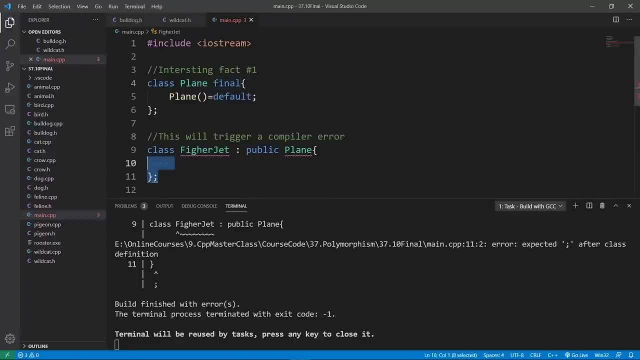 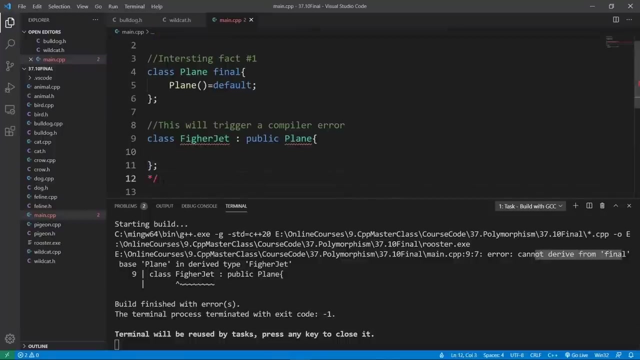 forgot to put our closing semicolon on our classic definition here, but we can build again and get our error. okay, the world is finished with errors and the error is going to be that we cannot derive from a final class. this is what we expect here. let's comment this out, because I just wanted you to see this. 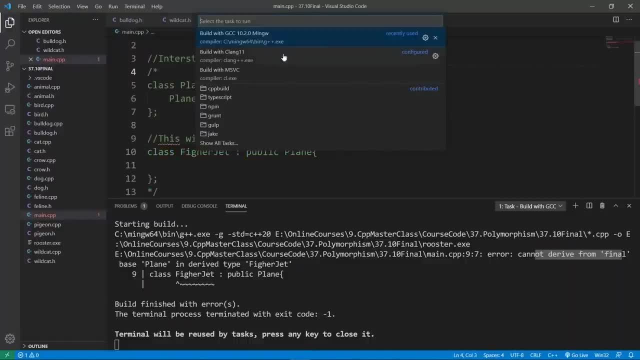 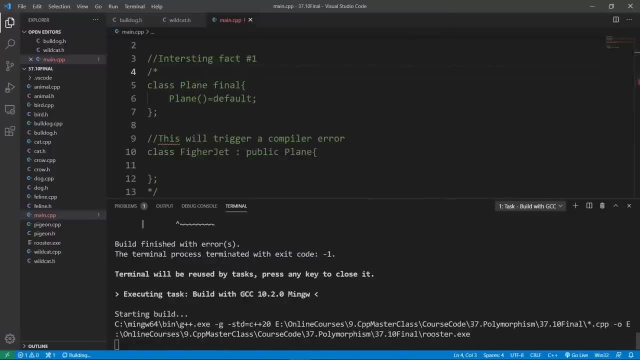 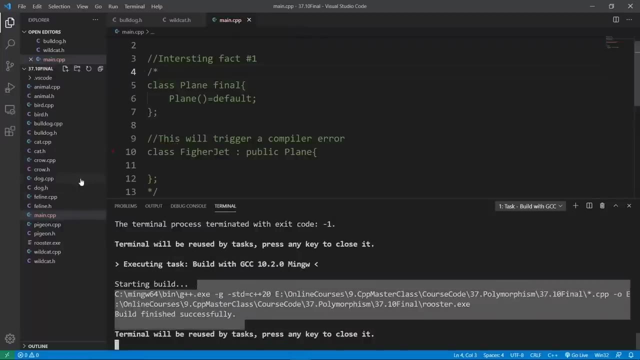 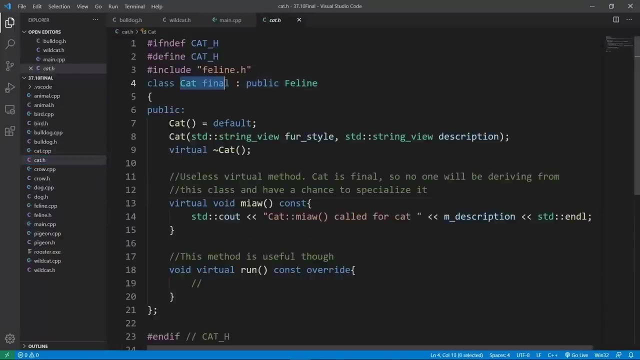 fact, another interesting thing c++ allows you to do is to set up a new virtual method in a final class. so let's go back to our final class, which is the cat class. if I remember correctly, this is a final class. we can't derive from this class, but we can set up a virtual method, for example, 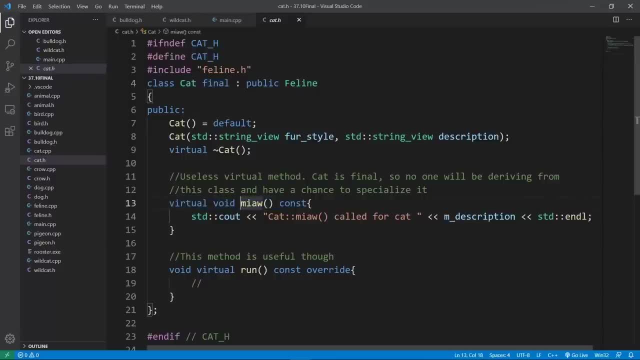 the virtual method here called meow, is useless. why is it useless? it is a virtual, and I'm marking it. virtual means that you at least want people inheriting from this class to inherit it and use it or, even better, you want them to have the ability to specialize or override this method. and 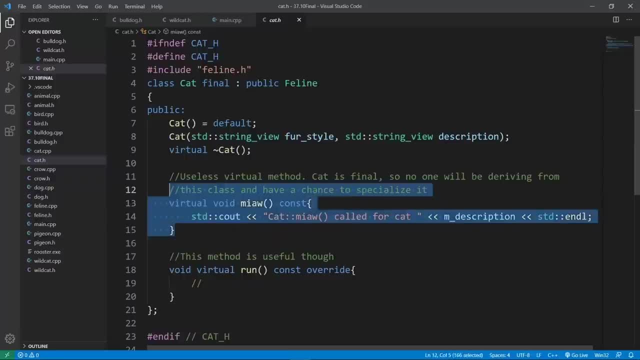 make it to do more specialized things, but you can't really do that because you can't derive from this class altogether. so this is something that c++ allows us to do, but this is a useless method which will never be used in any way. so this is something I want you to be aware of, but this is. 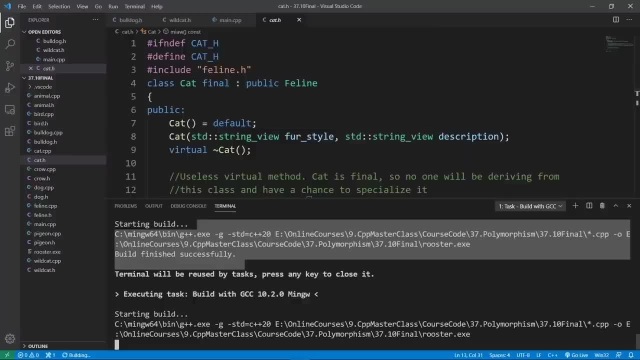 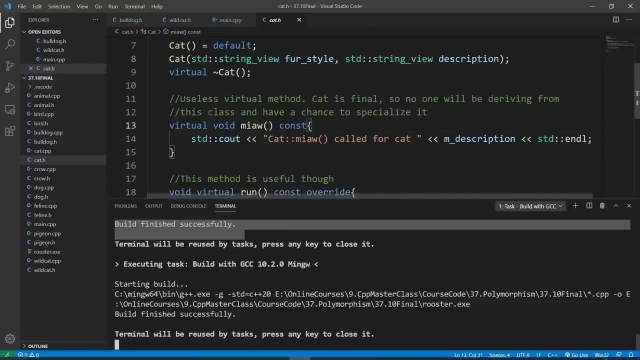 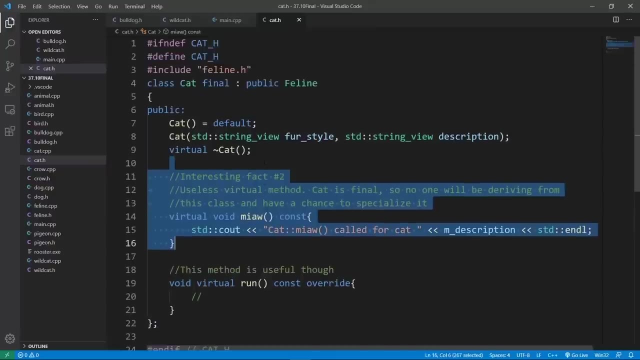 going to compile again. let's pass this through gcc. you're going to see that this is going to compile and work, even if is really useless. i want you to be aware of this. okay, so the world is good here. okay, so this is our interesting fact number two: okay, even if this method is useless, it is possible to specialize. 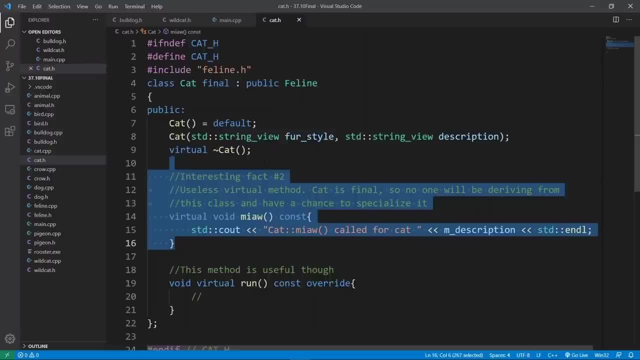 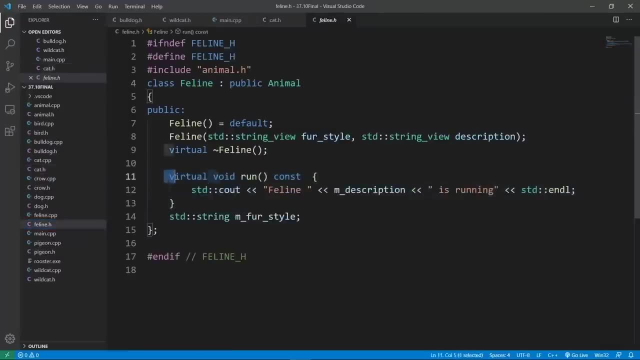 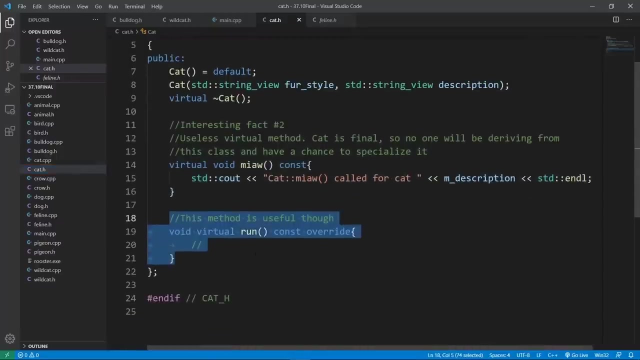 a method coming from upstream classes, from your final class. for example, in feline we have a method called run which was introduced there. i think we can override this method in our final class, which is the cat class here. so this method is going to be useless, because it will be. 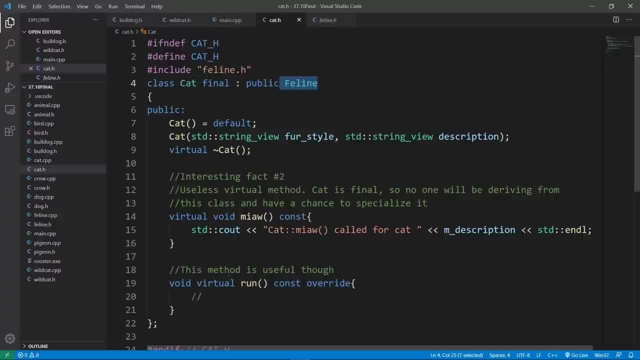 specializing what we get from our app stream class. this is going to work okay. so, since we are looking at a few useless things you can do with final combined with the virtual mechanisms in c plus, i want you to see that it is possible to set up a virtual method and mark it as a final in the same. 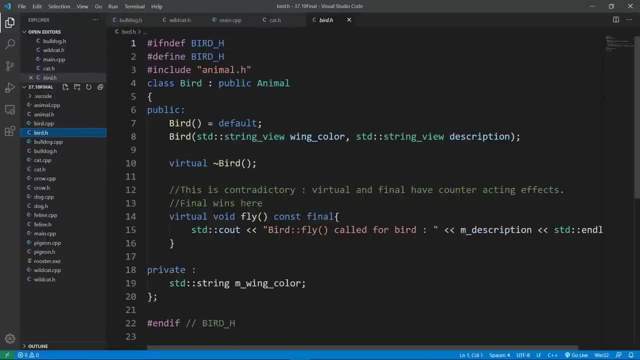 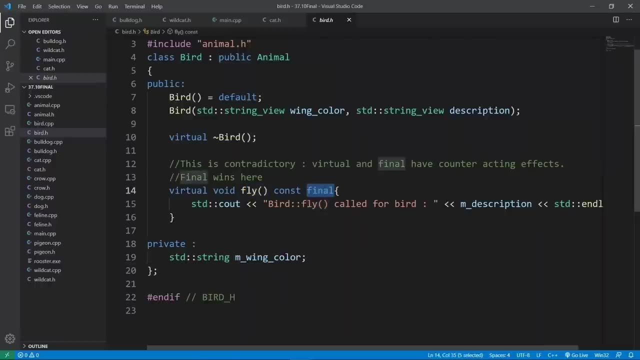 declaration and we're going to go to the bird class and really show you that frankly. example: we have a virtual method which is called fly, but this is marked final the moment we declare it and this is going to be contradicting. for example, the virtual keyword means that people. 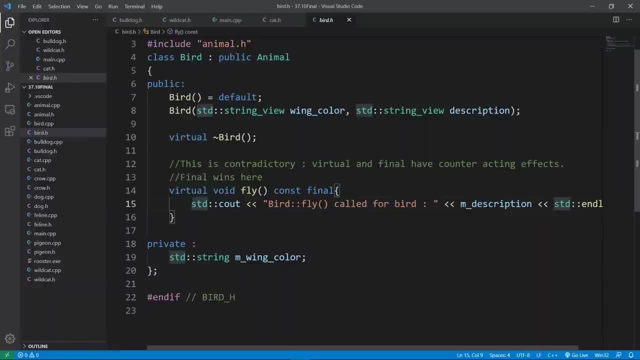 downstream will be able to specialize this or inherit this, but at the same time we are marking this guy as final. so we are saying nobody downstream will be able to override this method. if they do that, they will get a compiler error. now which one is going to win, virtual or final? 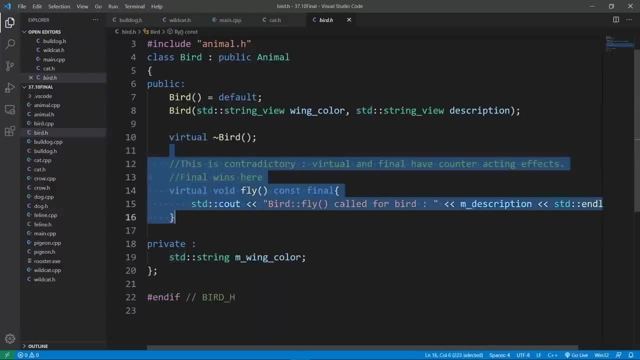 final is going to win because if you try to override this method in downstream classes, you will get a compiler error. let's go down and look at one bird we might have in our program, for example, we might have a pigeon. let's grab this method and try to override it. you're going. 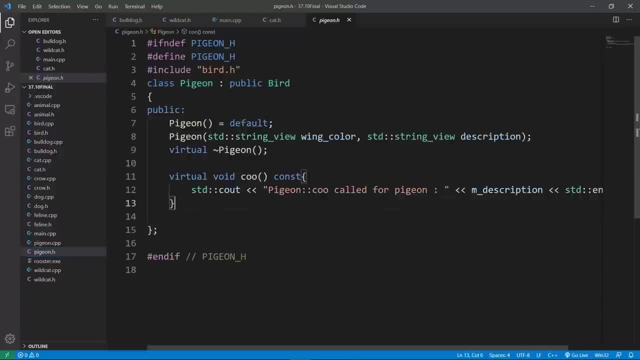 to see that we get a compiler error. we can go in pigeon and put in the fly method and, for example, we're going to say pigeon, fly here and i'm going to say override, we are trying to override this method, but we're going to get a. 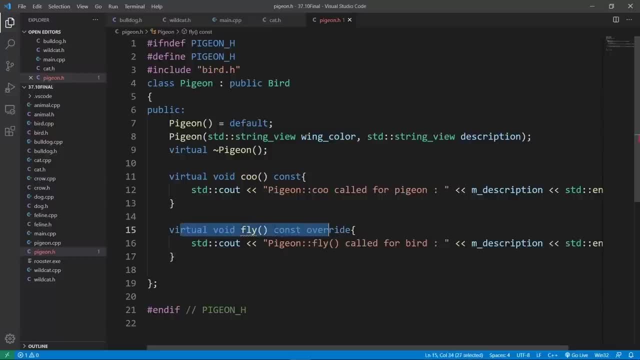 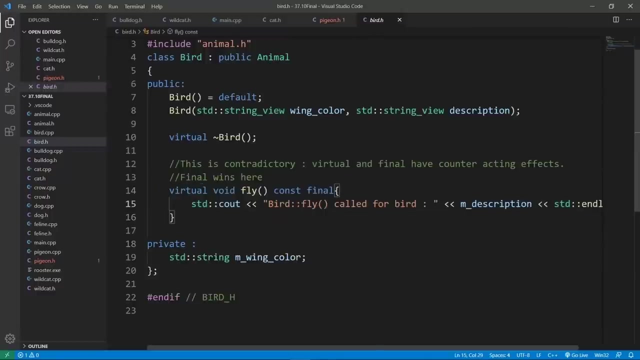 compiler error. you see, we have a squiggly line because this is a final method and we are trying to override this in a downstream class, and this class is a downstream class from bird and in bird we map this method as final. so this is not going to work. even if this is virtual you want to be. 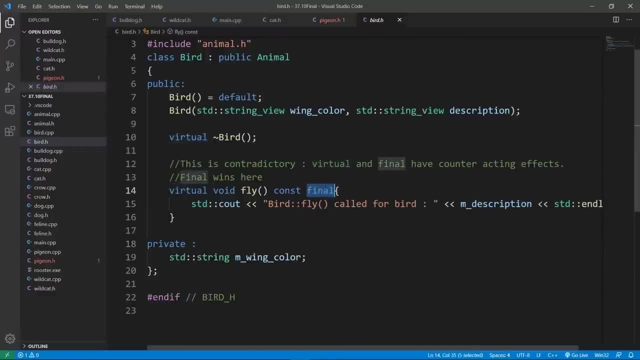 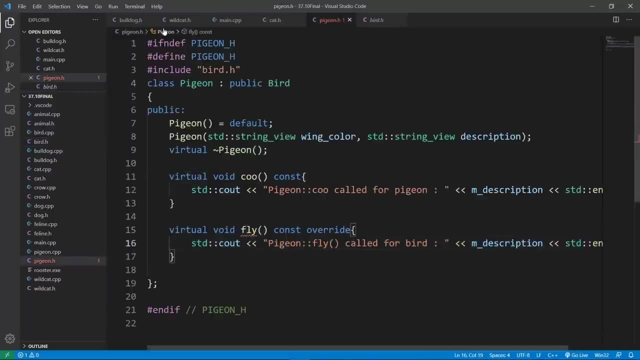 able to really use the virtual mechanism, because this is final. if we're trying to inherit from this, we are going to say, override this, and we're going to say, override this and we are going to. if we're trying to override this like we are doing in pigeon here, we will get a compiler error. 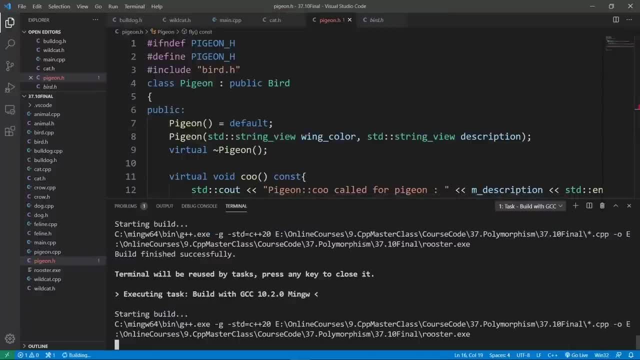 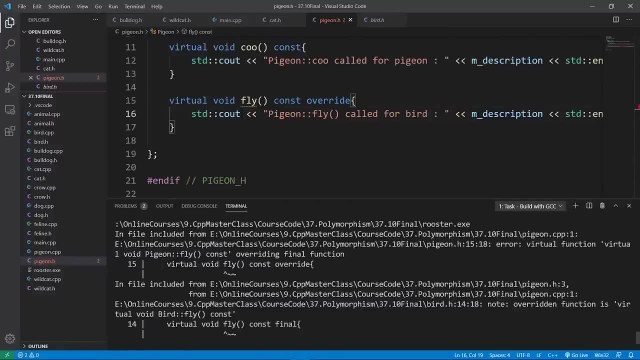 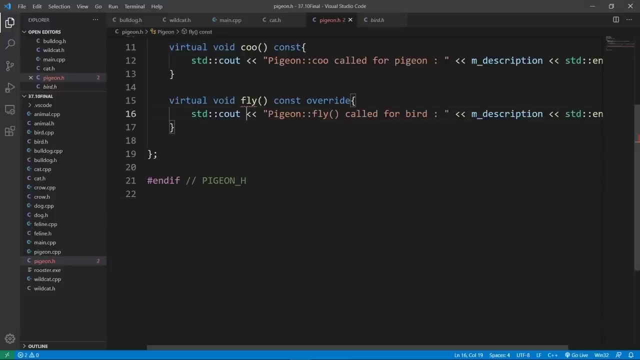 let's try and build our program and we will see that we get our trusty compiler error. the world is going to finish with errors and if we go up we're going to find our error. we're going to say: virtual function: fly overriding final function. we are overriding a final virtual method and this is. 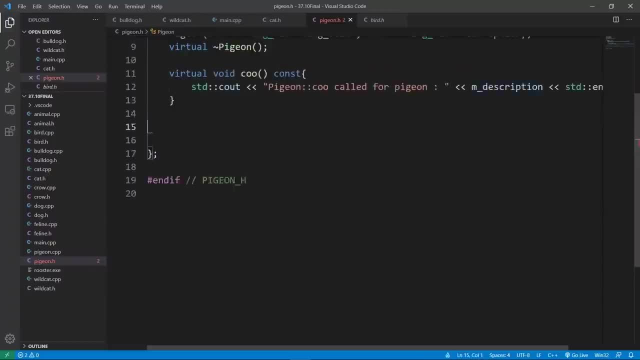 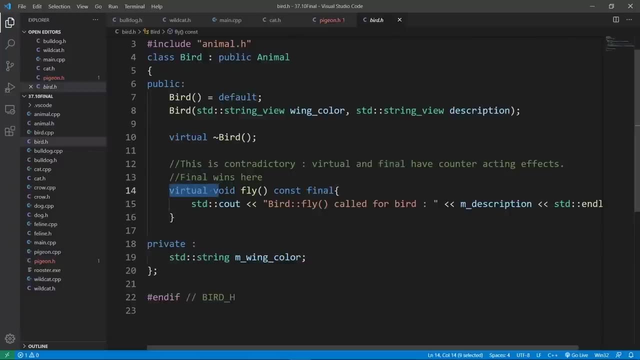 going to give us a compiler error. we can't do this. this is something you can't do in your c++ program. so this is really confusing, because in bird the virtual keyword suggests that you can really specialize this in downstream class. but this is contradicting and c++ allows you to do. 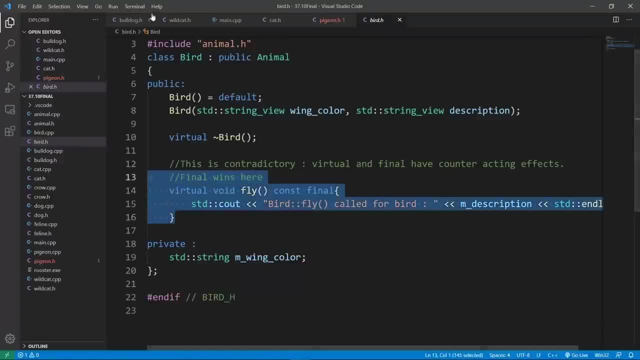 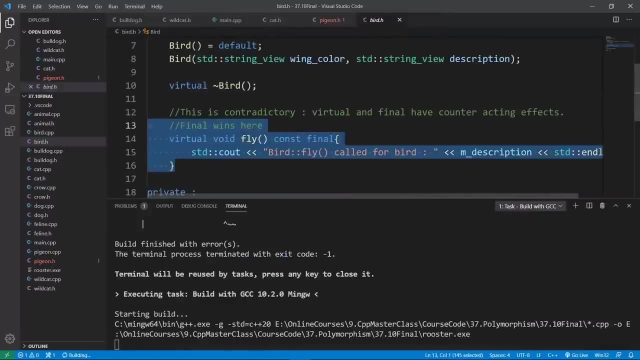 this. you need to be aware of this again. if we don't override this and leave this in, the code is going to compile, but in my opinion, this is really confusing and you need to be aware of this. that's the whole point of this lecture. here let's make sure the code is building, and this is really. 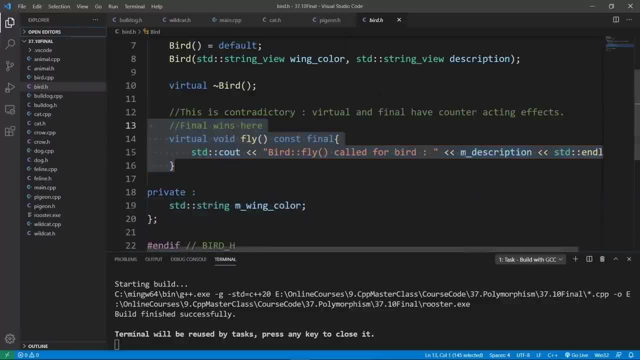 all i had to share in this lecture. you introducing the final keyword to you. you can use it to restrict how people override your virtual function, or you can use it to restrict people from inheriting from your class altogether. and use these things if they make sense for whatever application you are designing with c++. we are. 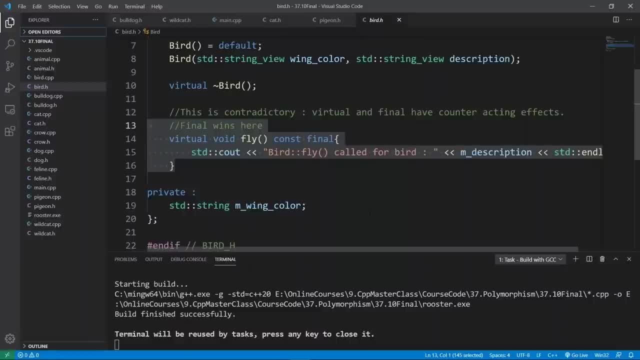 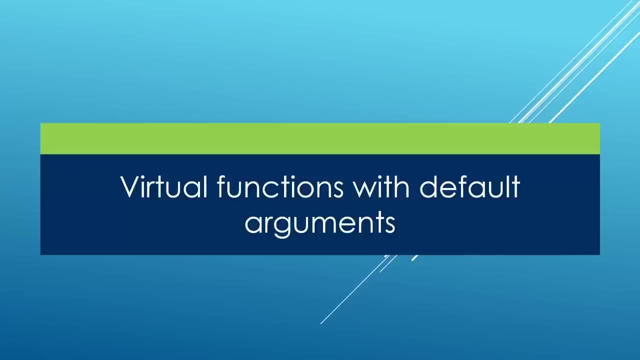 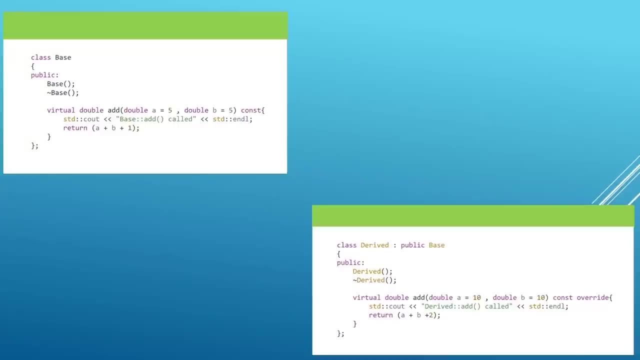 going to stop here in this lecture. in the next one i am going to show you a secret you probably didn't know, so go ahead and finish up here and meet me there. in this lecture, i'm going to show you a very simple one. this is an empty括 in the dictionary. we just wanted to see what we have. 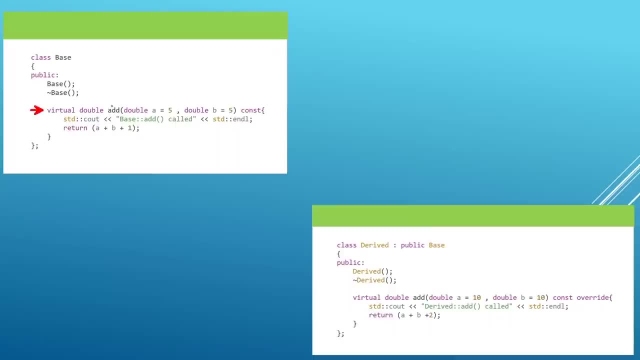 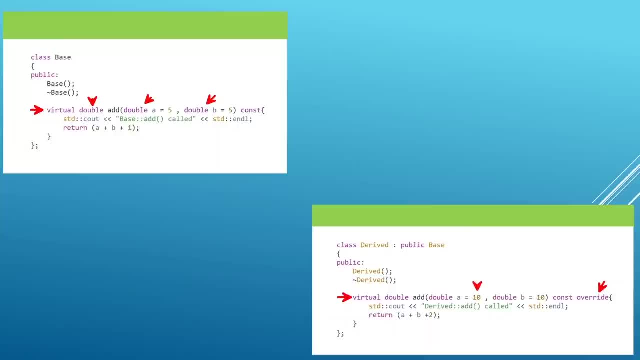 acting as our default parameter here. we are using 10 for a and b here and we want to see how this plays with polymorphism. now please note that with polymorphism, if we go through a base pointer to manage a derived class object, what we want is to call the most specific implementation of the 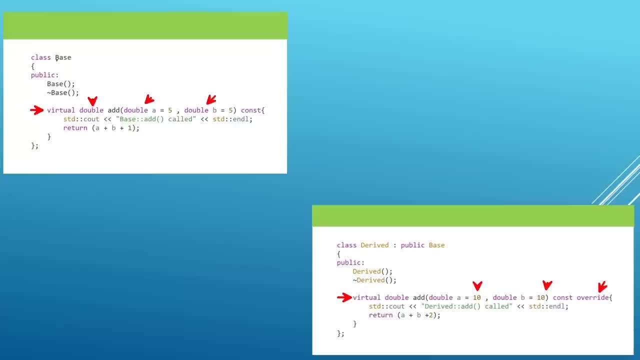 virtual function here. for example, if we have a base pointer managing a derived object and we call the add method from a base pointer, we will get the most specific method here called. but what you get with these default arguments is that the compiler is going to use static binding to decide. 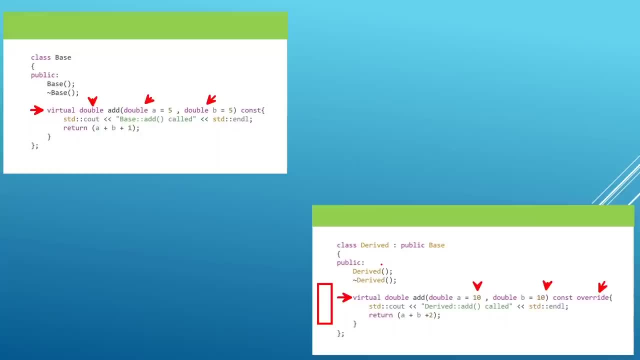 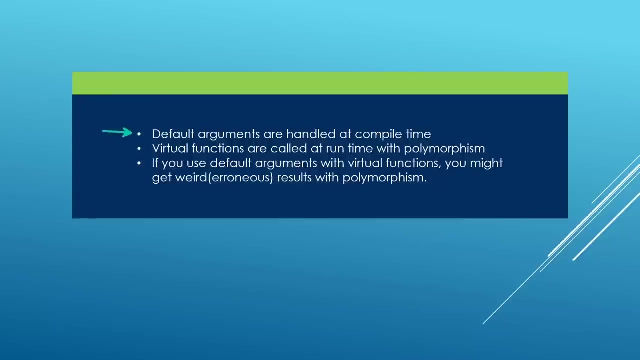 which default parameters to pass to your function. so even if you will get this method here called, the compiler will still use the default arguments we have in our base class. so we will call this method here, but we will use the default arguments you need to be aware of. okay? so another way to put this is that default arguments are handled at. 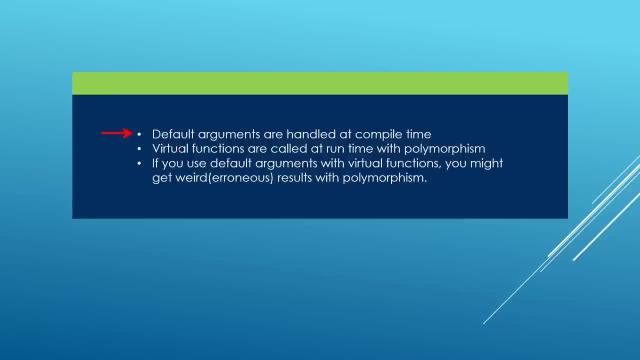 compile time. the compiler is going to wire these things at compile time, where you are building your application, and the virtual functions are called at run time with polymorphism. so if you use default arguments with virtual functions, you might get weird results with polymorphism because the default 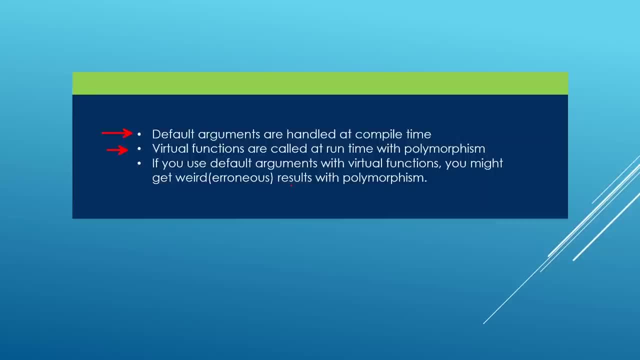 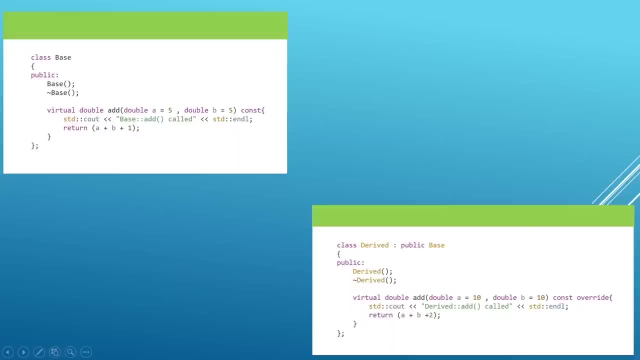 arguments you will be using are going to be the same as the default. arguments you will be using are going to be decided by static binding, but the actual function that you get called is going to be decided by dynamic binding. so we will call the virtual function in our derived class, but we will 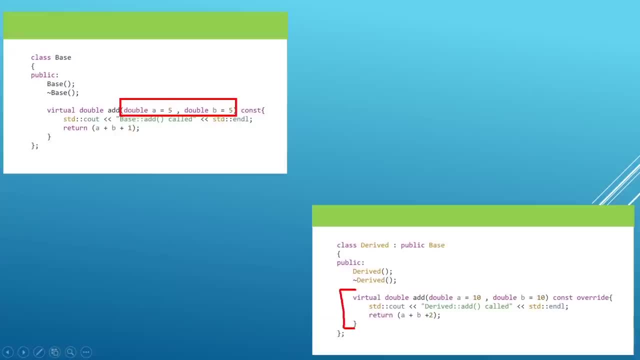 be using the default arguments from the base class. this is the behavior we'll get. you need to be aware of this and make sure this is what you desire. my personal preference is to not use default parameters or default arguments with virtual functions, because this is really going to make my code. 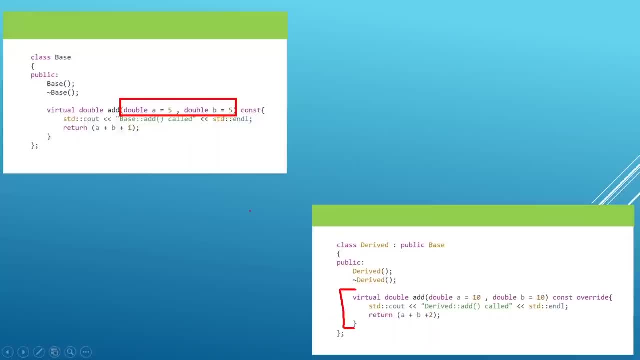 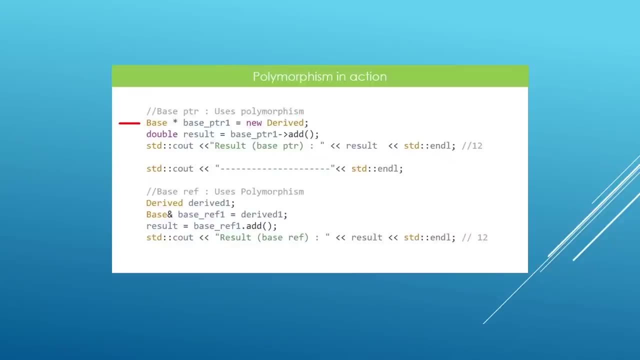 hard to follow and hard to understand, especially for other developers that might have to work on my code base in the future. okay, here is a simple example. we have a base pointer which is going to be managing a derived object, and we will call the add function here. what do we expect to get? 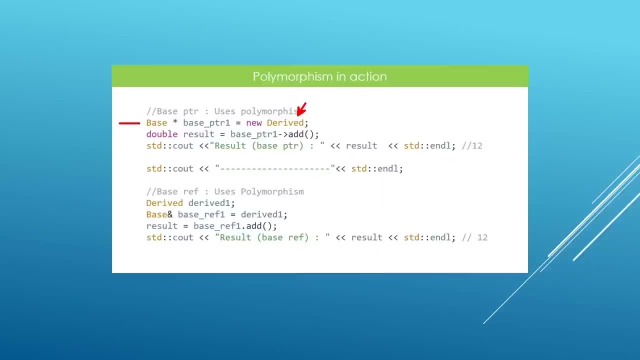 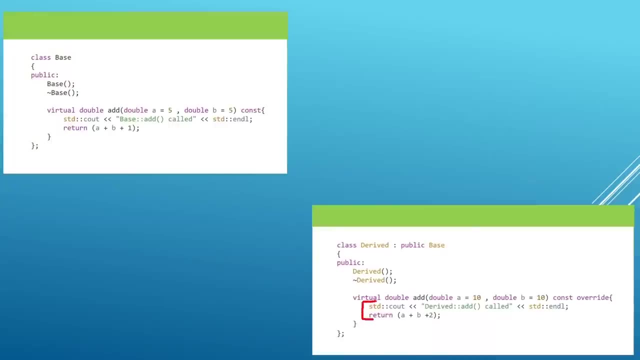 well, because we have polymorphism here, we will call the most specific add function here and that's going to be the add function from our derived class. but the default argument we passed are not going to be decided by the derived class. the default arguments are going to be: 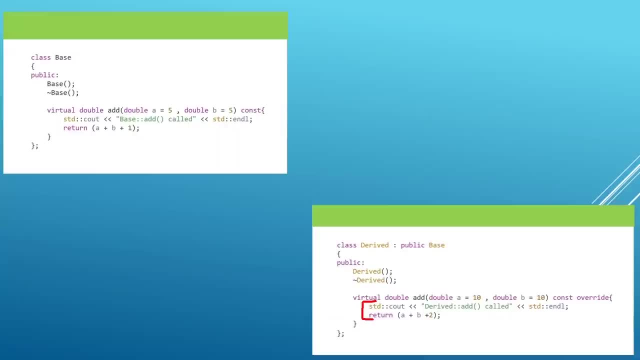 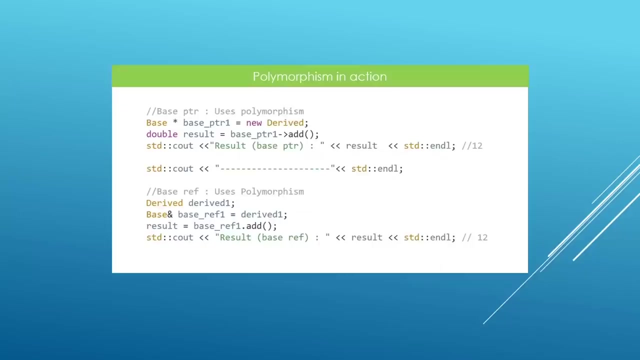 plugged in at compile time using static binding. so because the base pointer is a base object, we will be using the default arguments from the base implementation of the add method. so we will just plug in five and five. so we will add five to five and add it to. that's why we get a 12 right here. 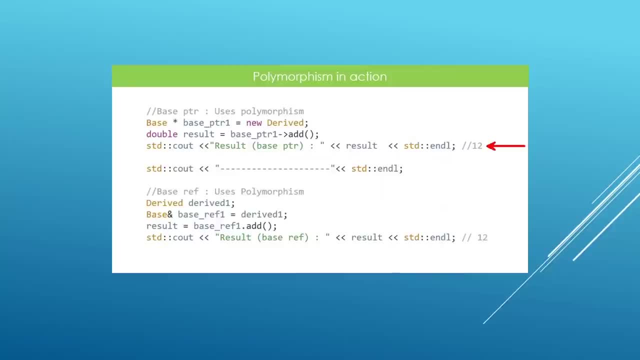 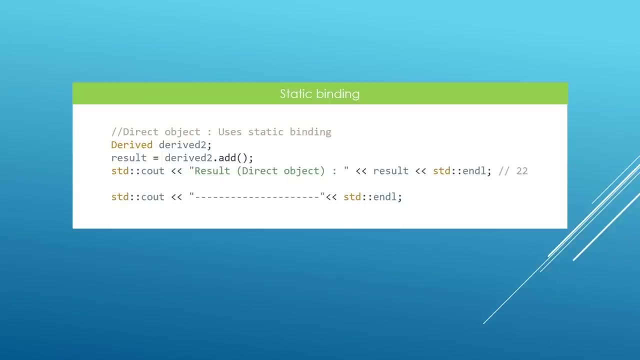 and if we go through base references, we will get the same result, because this is going to enable or trigger polymorphic behavior in our c plus plus programs. if we go through direct objects, we will be doing static binding and we will use the default arguments or default parameters from 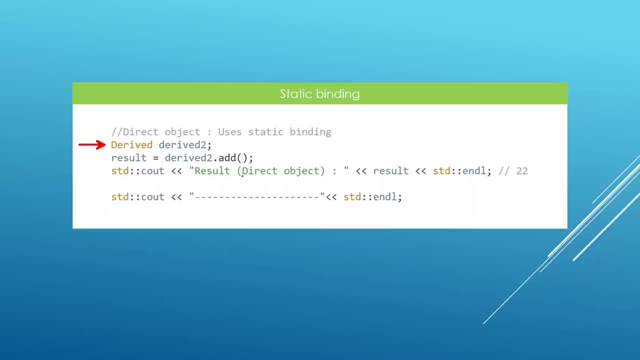 our derived object and remember that we use the value of 10 in there. so we are going to add 10 to 10 and add a 2 and we are going to get a 22, as you see here, through static binding, if we do slicing by. 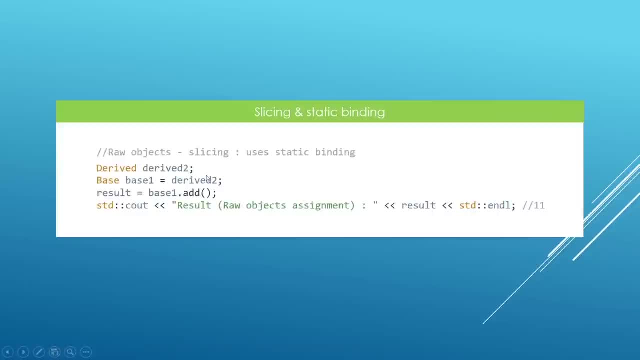 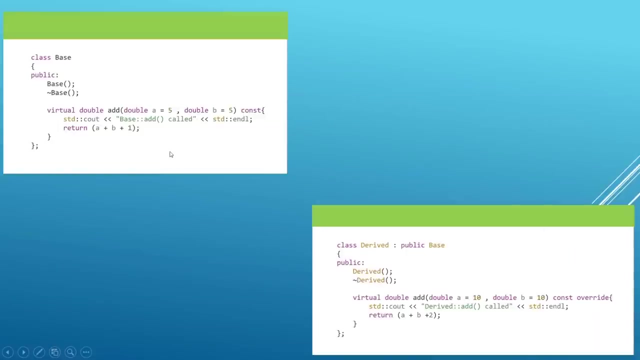 assigning a derived object to a base object. the derived information is going to be sliced off and if we add, we will use the default parameters from the base class and we will use the implementation in the base class. so if we come back to our code here, we will use the default arguments from the base class and that's a five. 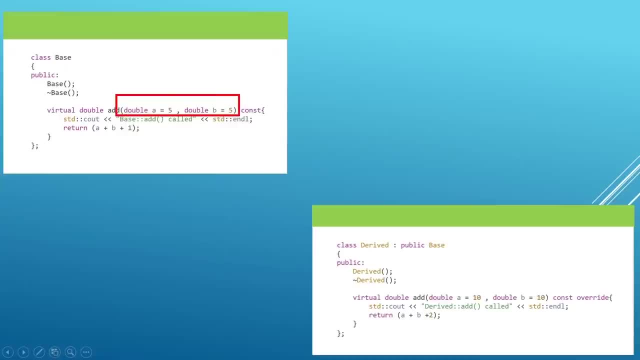 and a five. we're going to add them up because the body is going to be from the base class. remember, the derived information has been completely sliced off. so we are going to add a five and a five and one and we're going to get a two. 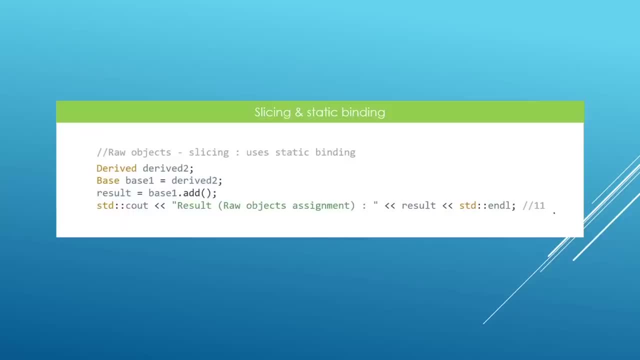 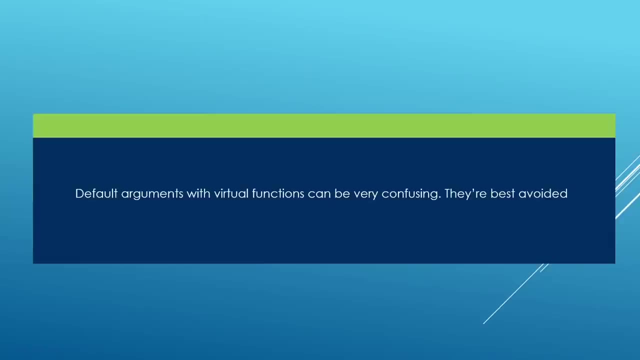 and we're going to get 11 printed out if we do slicing, and that's the result we get right here as a closing note before we head over to visual studio code again, default arguments with virtual functions can be very confusing. they are best avoided because they really are going to give. 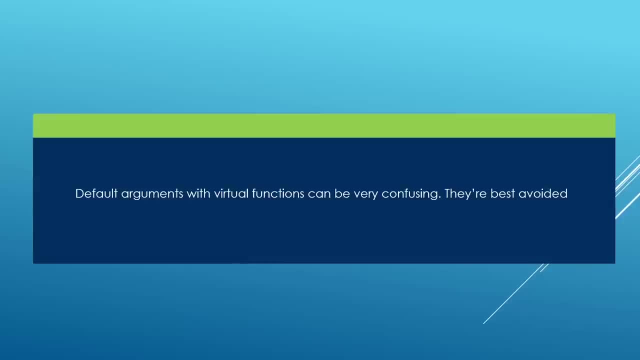 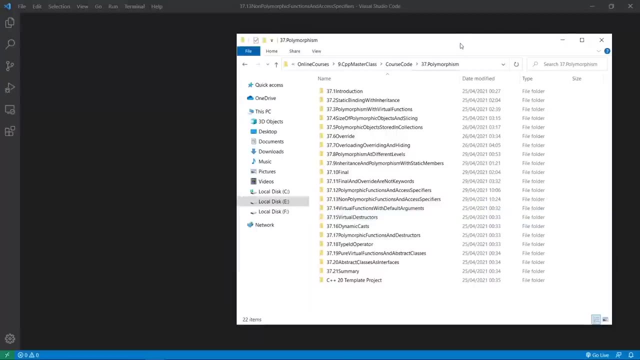 a hard time to anybody that is going to be working on your code in the future. now that you know this, we're going to head over to visual studio code and play with this a little more. here we are in our working folder. the current project is virtual. 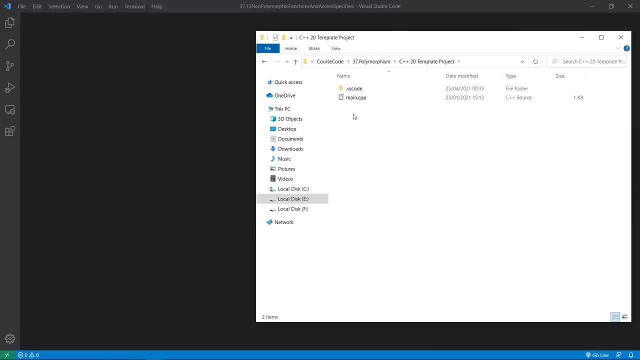 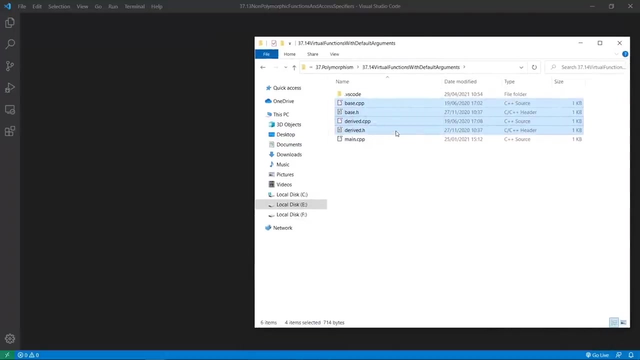 functions with default arguments. we're going to grab the code from our template project, we're going to copy this and put this in the current project, and i am going to grab my classes base and derived that we are going to be using here. if you don't want to type along, you can grab the source code from. 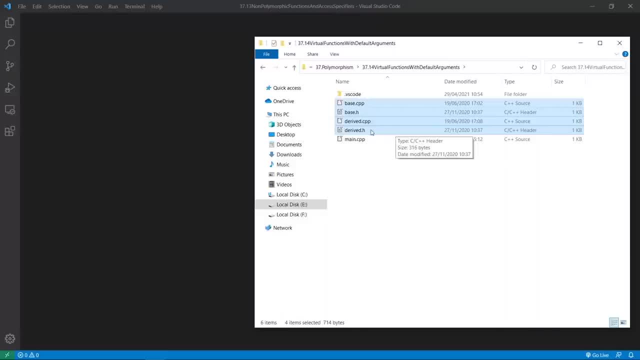 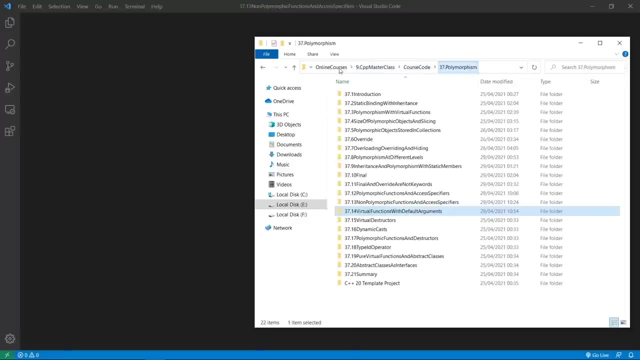 the resource section of the course. if you don't want to type all these classes or create them, you can grab the source code from the resource section on this lecture. you're going to download this and use this. you don't have to waste time typing these things, because many of these things are already familiar. 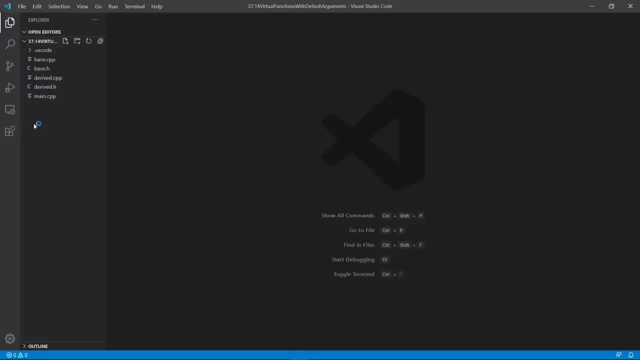 to you. we're going to open this in visual studio code and we're going to have our classes here. we have a base class which is going to have a virtual function with a pair of default arguments. here we are using five, five in our add virtual function here and if we go in derived, it is going to derive. 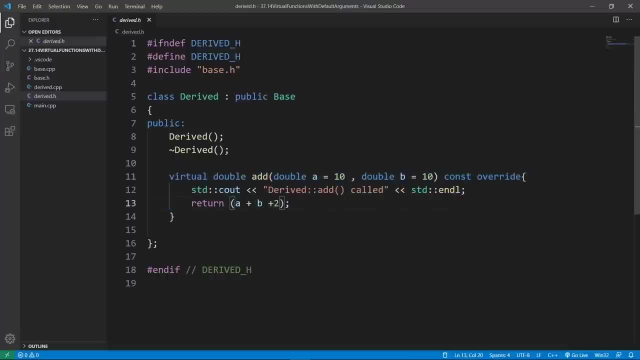 publicly from base and it is going to override our virtual function here. but notice that it is going to set up its own default parameters. so if we do polymorphism and use a base pointer to call the add method here we will get to the most specific or the most specialized version of the 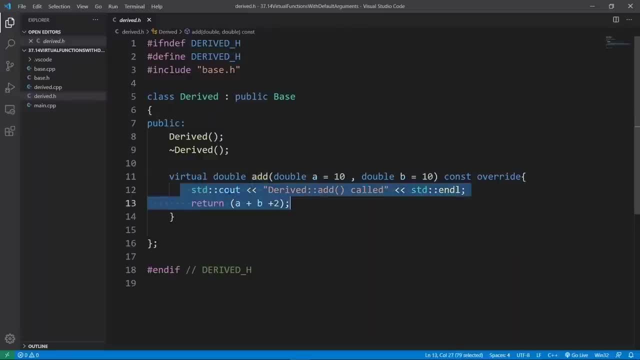 add method called, and this is going to call this body here, but the parameters are going to be decided by static binding. so, because we will be going through a base pointer, we will use the default arguments from the base class. that's going to be five, five and we're going to play with us and see what this is going to give. 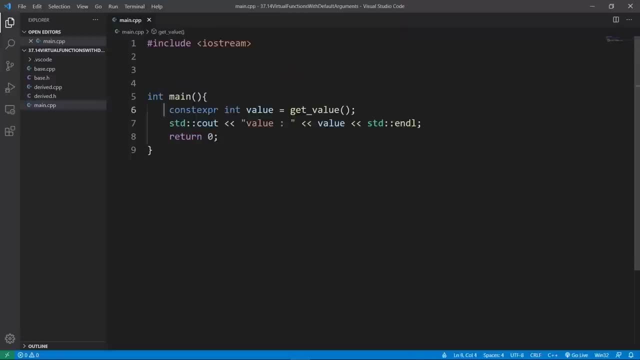 us in the main cpp file. here let's clean up a little bit. we're going to remove whatever we don't need here and we are going to include our derived class. we can do that. we are going to put in our code to really play with us. let's remove these spaces because we don't need them. we are. 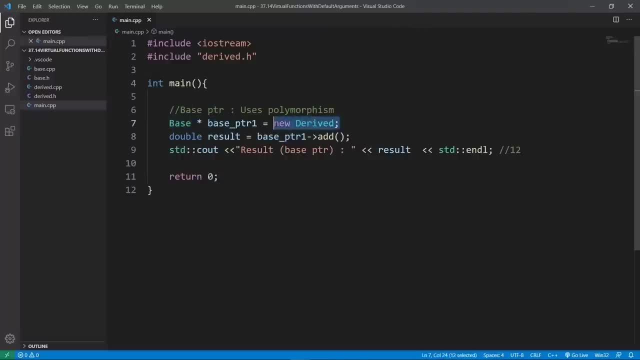 going to go through a base pointer and we are going to put in our code to really play with us to manage a derived object, and this is a setup we can use to put things in place here. we are going to call the add method. notice that we are not passing in any parameter because we are going 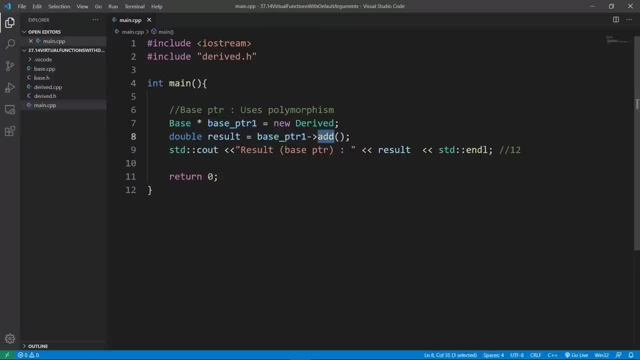 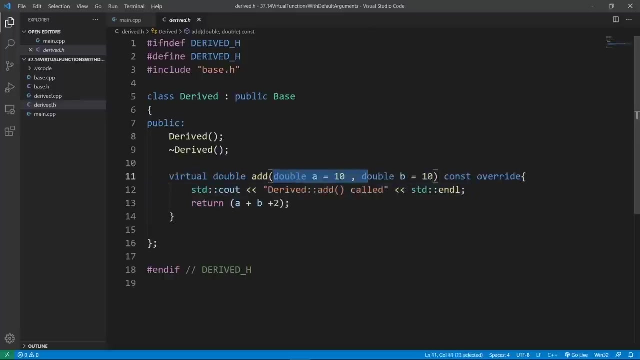 through a base pointer and the add method is virtual, polymorphism will kick in and we will get the derived version of our add function called. so we will call this add function here, but be careful, because we won't be using this default parameter here. so we are going to call. 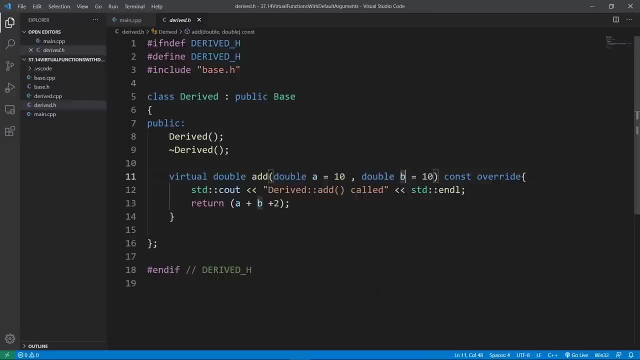 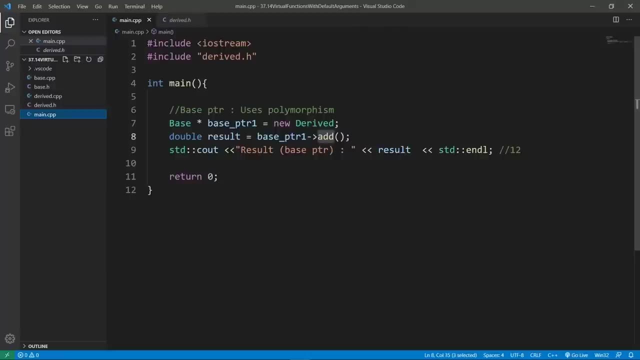 the add function and we will get the default parameters here. if we did, we would add a 10 to a 10 and get a 22 in our main function here, but that's not going to be the case. the compiler is going to use static binding to decide which default parameters to use, either those in the 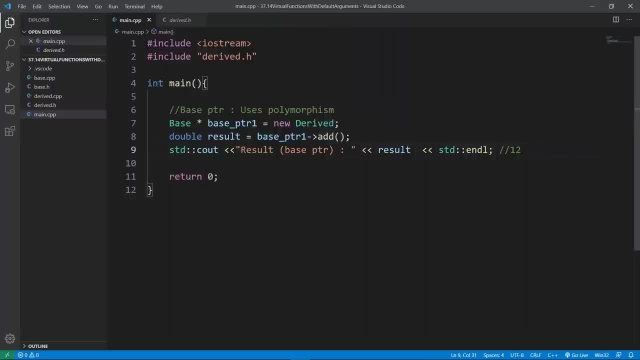 base class or those in the derived class, and notice that if we hover over this add function, you see that the compiler has plugged in those from the base class and that's what the compiler is going to do. so it is going to add a five to a five and it is going to add a five to a five. 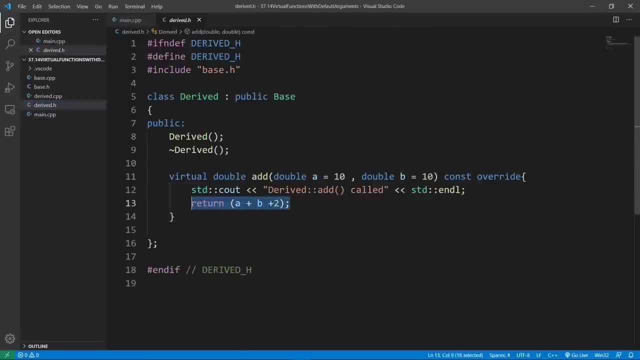 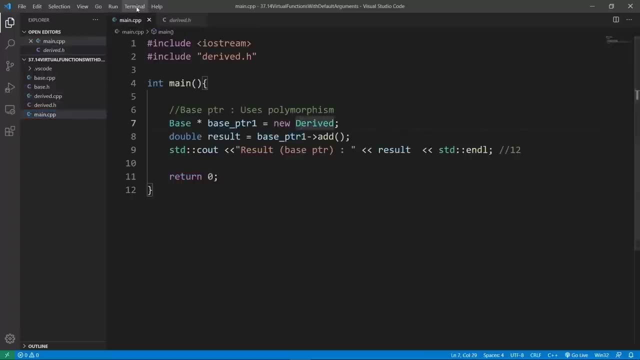 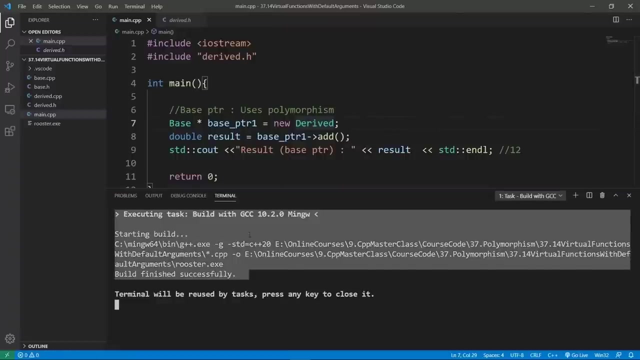 to add two to that. i think that's what we are doing in our derived version and we are going to get a 12 printed out. let's build and see if this is actually the case. we're going to pass this through gcc and that's the compiler. that is our favorite. now the book is going to be good. 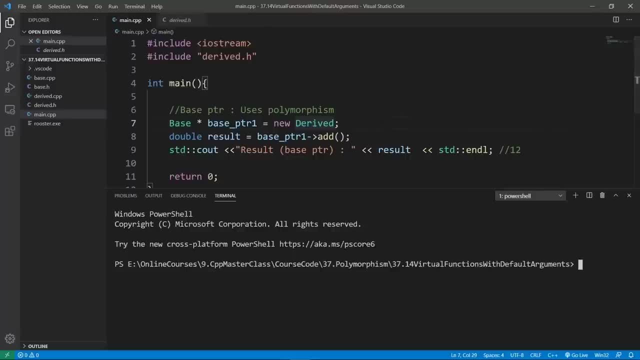 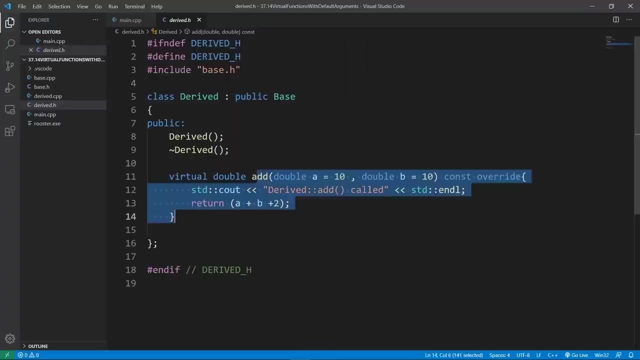 we can close this and bring up a powershell window and if we run rooster, we're going to see that derived ad was called and the result was 12. here this is what we get again. the compiler is going to call the most specialized virtual function override here, but it is going to 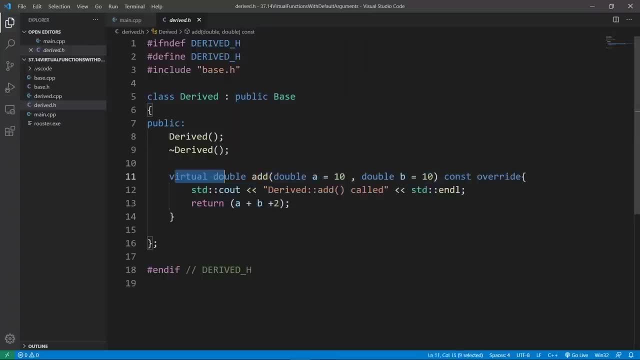 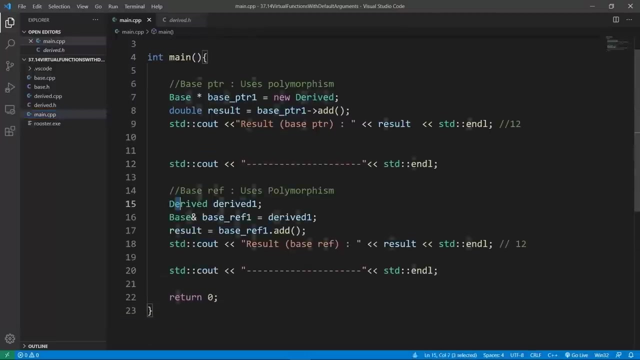 use the default parameters from the base class. you should really know this and this can really be confusing, especially if you are a beginner to polymorphism. if we go through a base reference, we will also get polymorphic behavior. so if we have a derived object and we set up a reference, 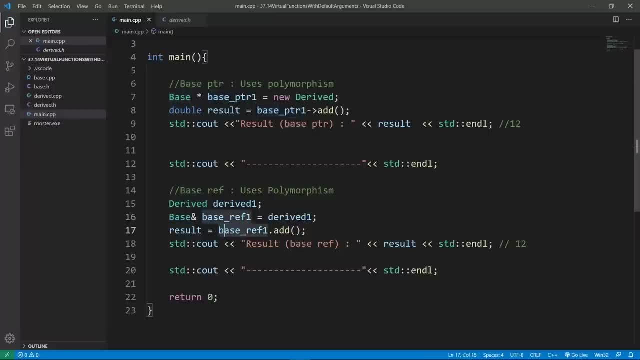 to that which is of type base and we go through that base reference and call the add method, we will get the most specialized ad version called, so that's going to be derived add. but we will use the default parameters from the base class, because which default arguments we use is decided by using static binding and 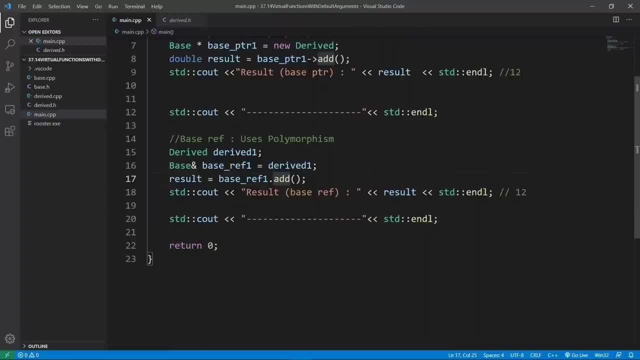 that's what we get here, and a visual studio code is really helpful here, because if we hover over the add function, we're going to see which default parameters were plugged in by the compiler and you see that the ad function is going to be derived from the base class. and we're going to see which default parameters were plugged in by the compiler and you see that the 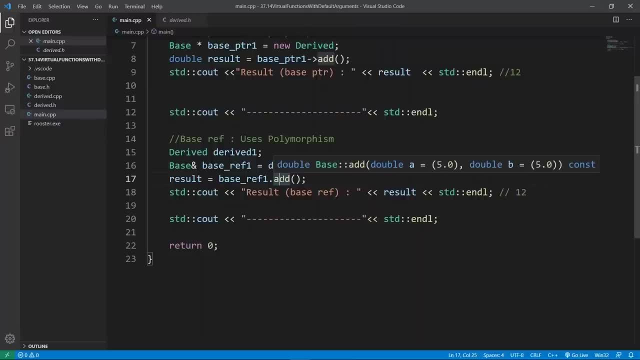 are those from the base class. so we are again going to add five to a five and we are going to add a two and we will get 12 printed out here. if we build and run, we're going to see that this is the case. the build is good, we can clear and run rooster. we're going to see that. 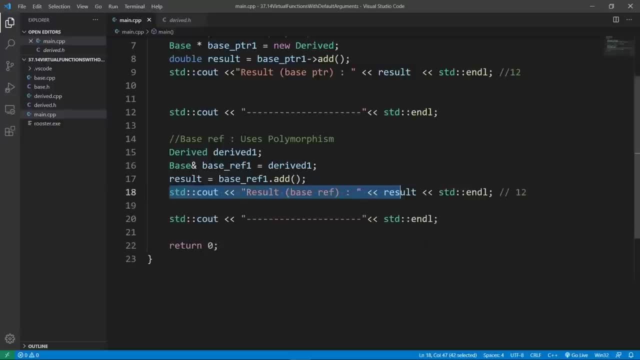 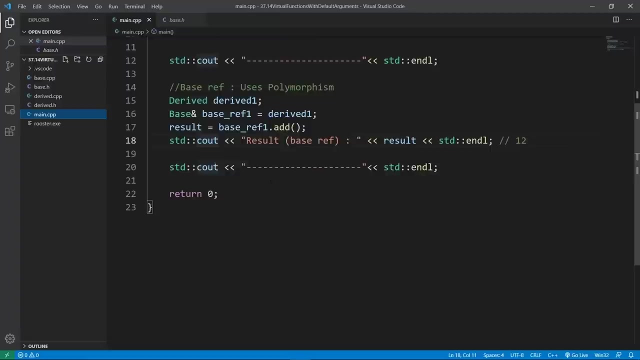 with a base reference. we're also going to get a 12.. we will get the most specific implementation of the add method called, but we will plug in the default parameters from the base class. i really wanted this to be super clear. if you set up things in a way that you are going to 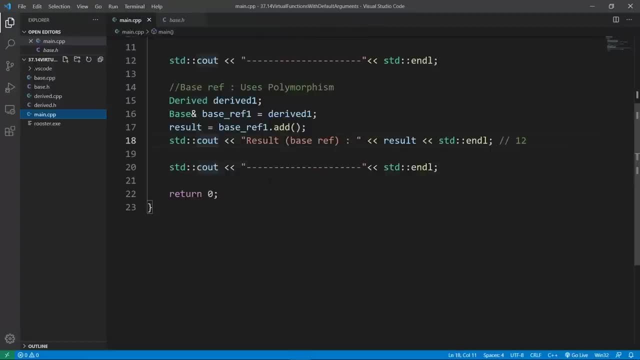 get static binding, then if you are going through a base object, you will call the base version of the add method and you will use the default parameters from the base class. if you happen to be manipulating a derived object, you will use the information in the derived class, the derived version of the 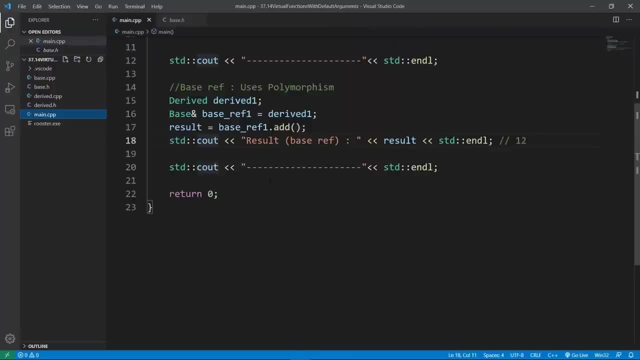 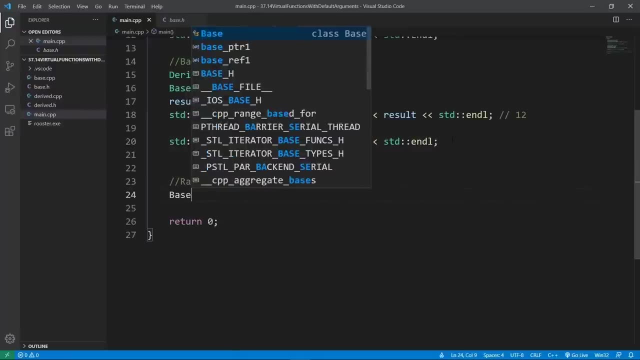 add method is going to be called and we are going to use the default arguments from the derived class. so if we set up another example here, we can set up a base object, for example. we're going to say base and say base three. we can do that and we try to call the add method. we can say base three. 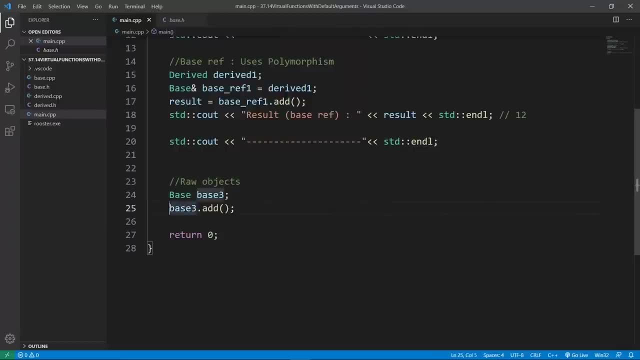 and say: add, we can try and store this in our research variable and we can print this out. we're going to say sdbc- out row research. we can say something like this and we're going to print out the result here. if we build and run, we're going to see that this is going to call. 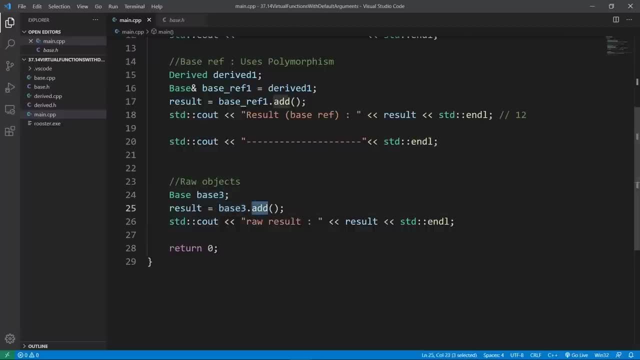 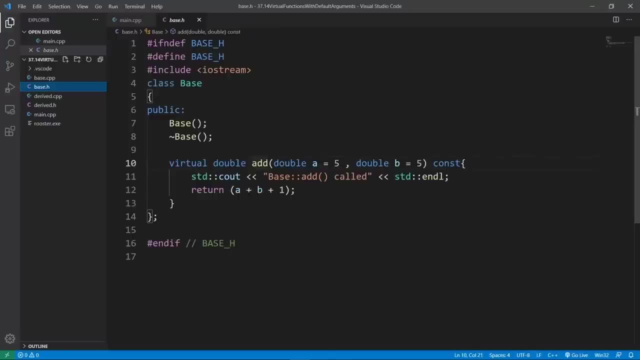 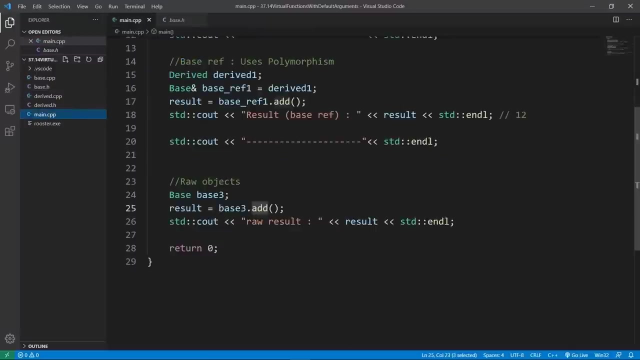 the base version of the add method and it is going to use the default parameters from the base. if we go back to base, we're going to see that we are going to add a 5 to a 5 and we will get 11 because we will plug in a 1 and return the result here. let's build and run and see that this is. 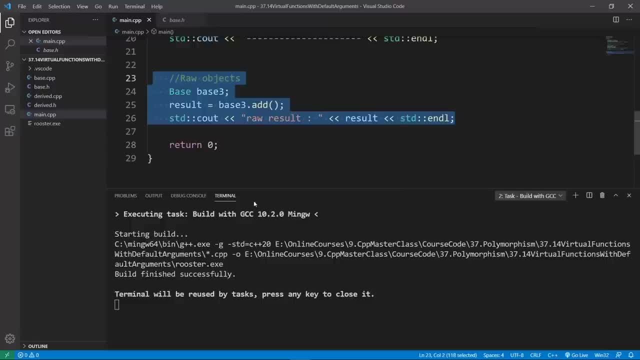 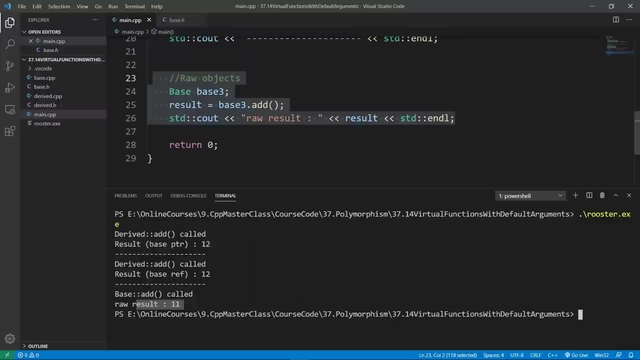 actually the case. so this is going to be completely doing static binding. let's clear and run. you see that the build is good, we're going to run the restaurant and we will get 11 printed out here. so if we run, it will show us that the build is good and we're going to run the restaurant and 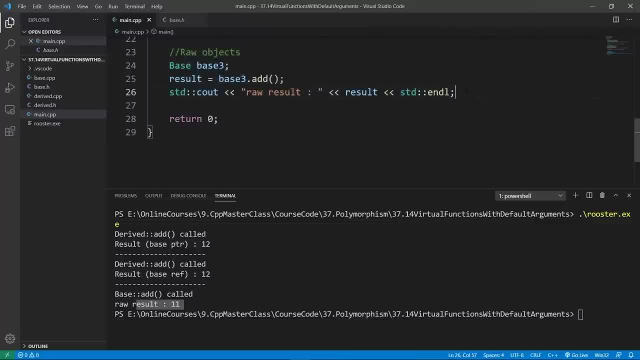 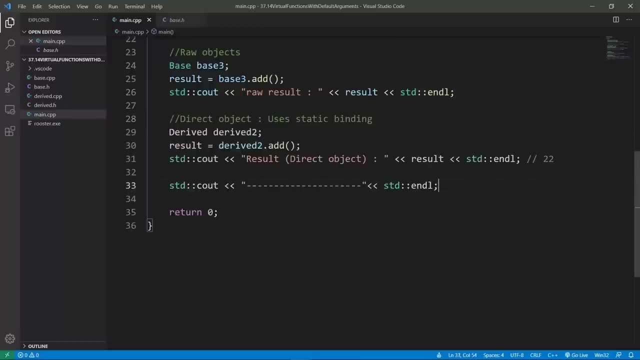 we're going to get 11 printed out here, so this is going to be completely done. so we can see this: if you assign a derived object to a base object, you will get slicing. let's see that we can actually do this. but before we do that, i also want you to see that you can also do row direct objects of. 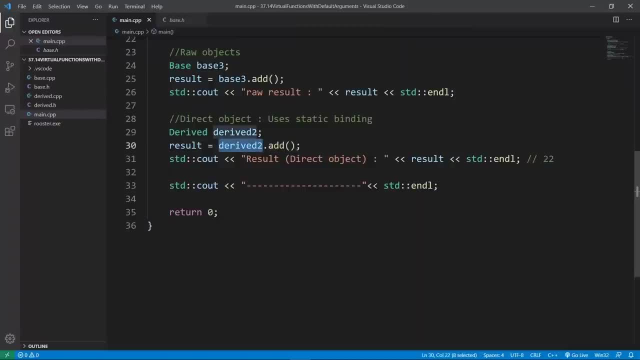 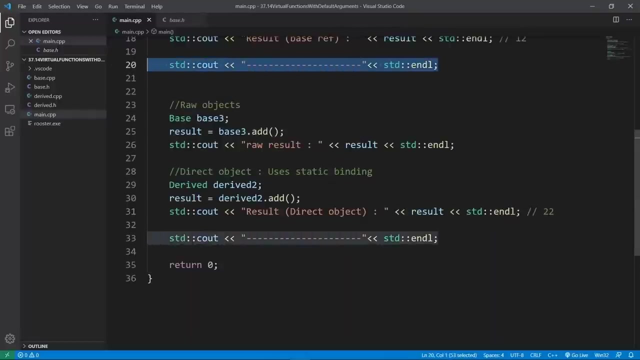 derived classes. if you do this, you will get the information from the derived class, we will use the add a 10 and we will add a 2 to that and we will get a 22 printed out. i think we can do this, so let's put in a separator, because that's going to make it easier to follow these things. 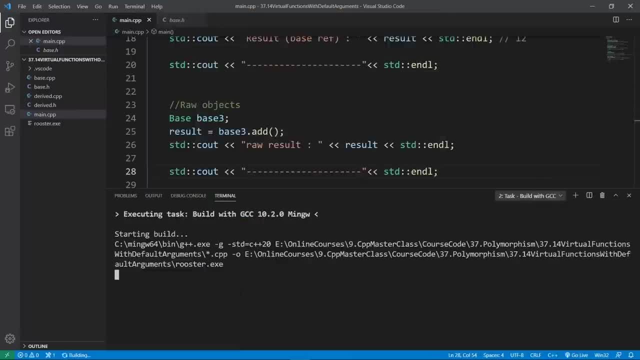 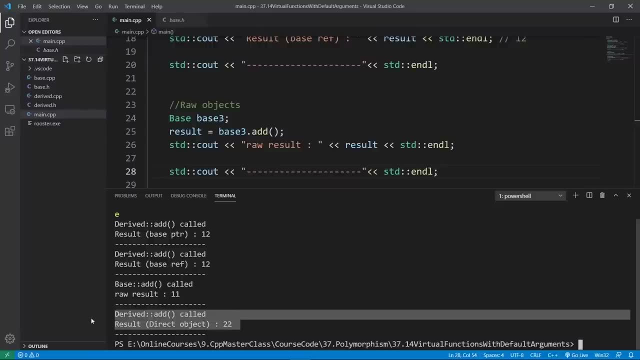 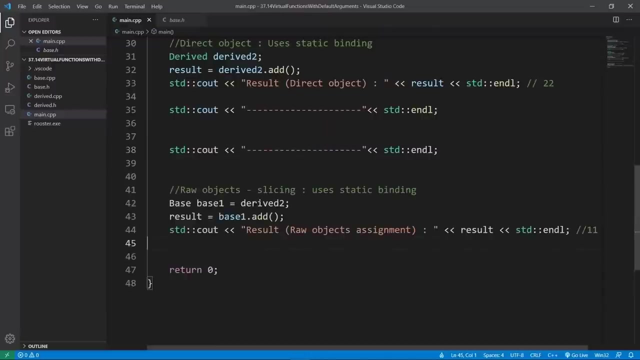 and we're going to build with gcc. the build is going to be good, hopefully. the build is good. we can clear and run rooster and we're going to see that we get a 22 here. if we assign a derived object to a base object directly by doing something like this, i think we don't need 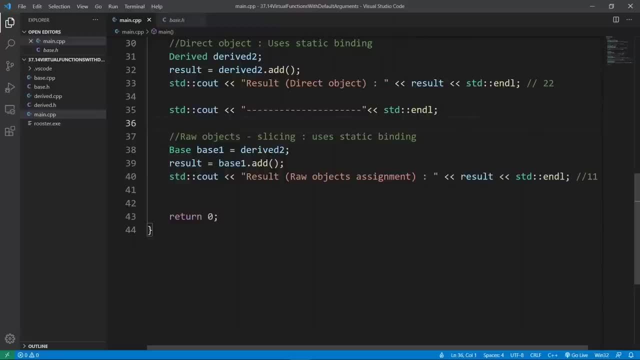 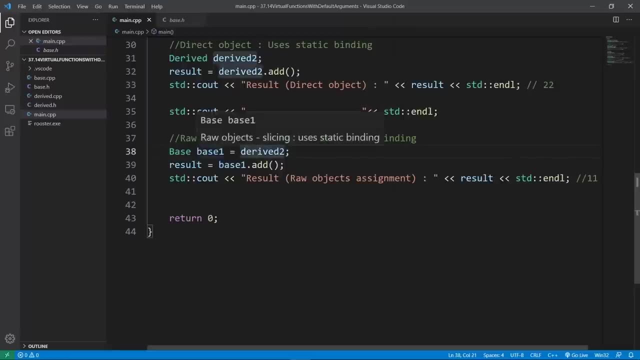 this guy here. you can remove this. we have a base object that we are setting up here and we are assigning a derived object to this base object here. if we call the add method, we will get the version from the base class because, mind your steps, this is going to slice off all. 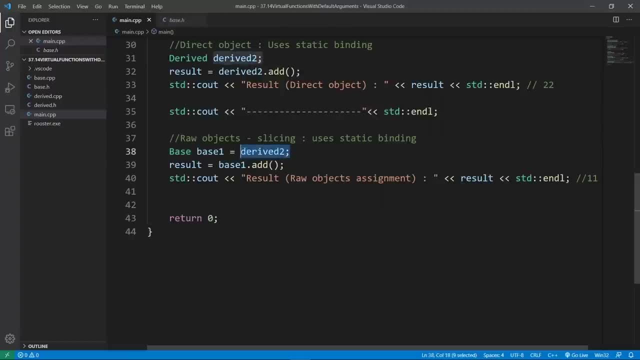 the derived information because we are not going through any kind of base or reference. so this is going to slice off all the information we have in the derived object here and we will be left with the base information. and if we call the add function here, you see that we are using. 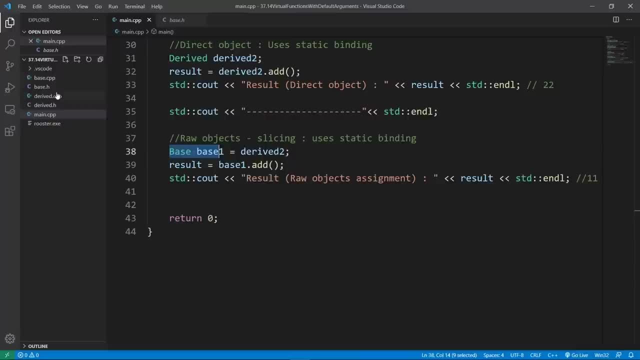 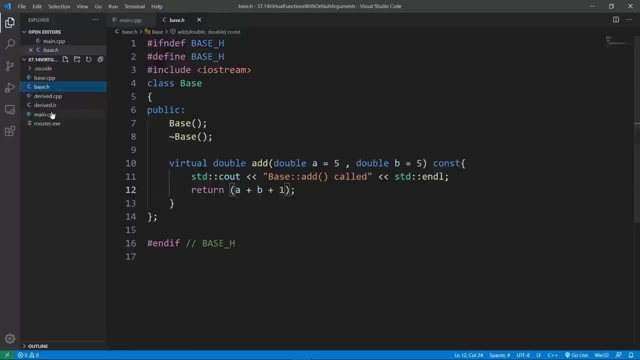 the default parameters from the base class and we will use the body of the base class implementation here. so we will add a 5 to a 5 and we will add 1 to that and we will get 11 printed out as we see here. let's build and actually prove this. we're going to pass this through gcc. 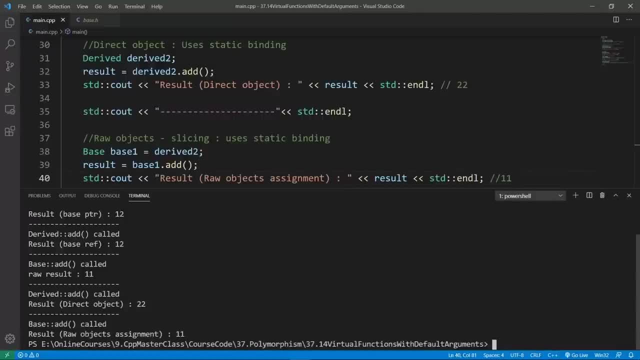 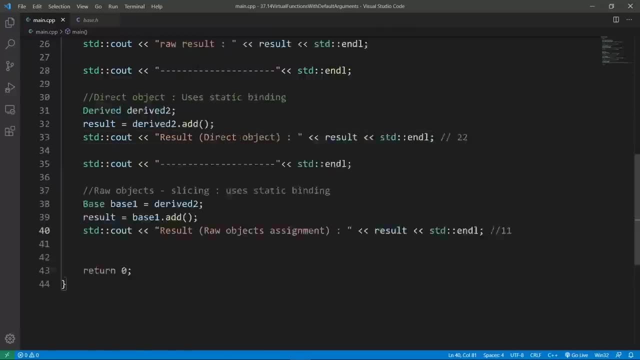 the world is going to be good. we can clear and run rooster and we are going to see that the result is relevant if we do row object assignment here. this is really all i wanted you to see in this lecture: that you should really be careful if you are using virtual functions. 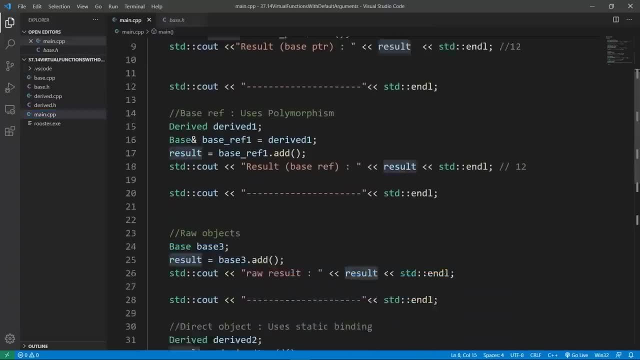 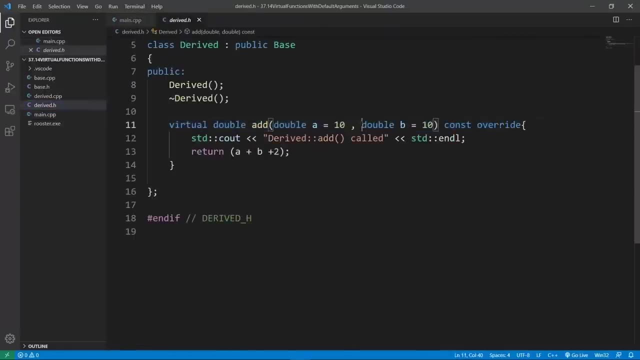 mixed up with default arguments. the compiler is not going to do dynamic binding on the default parameters. it is going to decide which default parameters to plug in at compile time using static binding. so the compiler is basically going to look at the type of the pointer or object that you have and it is going to use that to decide which default parameters to plug in. 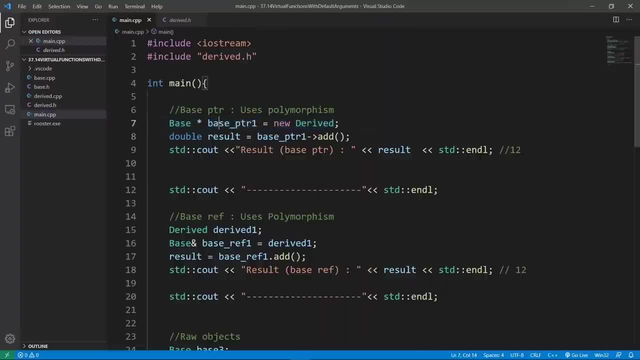 so at this example here, for example at line 7, it is going to see: what kind of pointer do i have? i have a base pointer, so i am going to use the default parameters from the base implementation and if you hover over here, you're going to see that it is going to plug in a five and a five. 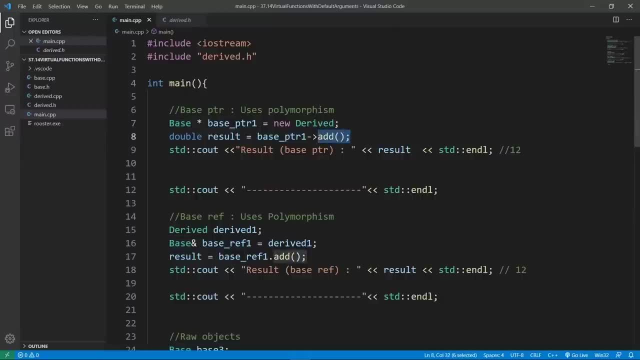 even if we are using the most specialized ad version in our inheritance hierarchy, the compiler is going to still use the default argument from the base implementation. down here on line 16, the compiler is going to say: which kind of reference do i have? it's going to say base. 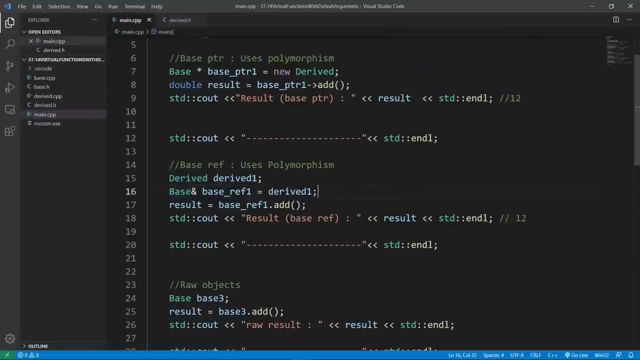 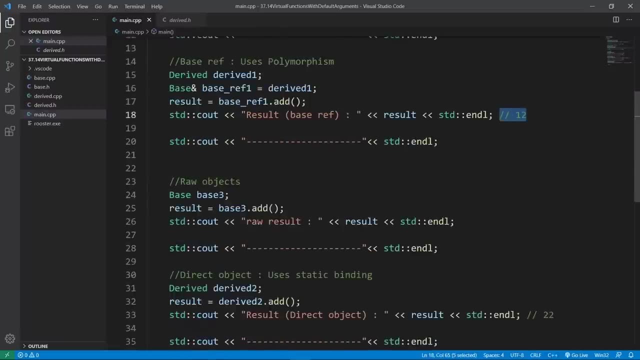 because that's what we have here. so it is going to use the default parameters from base and that's what it is going to plug in here, 5 and 5, and we're going to get this research here. down here on line 25, the compiler is going to 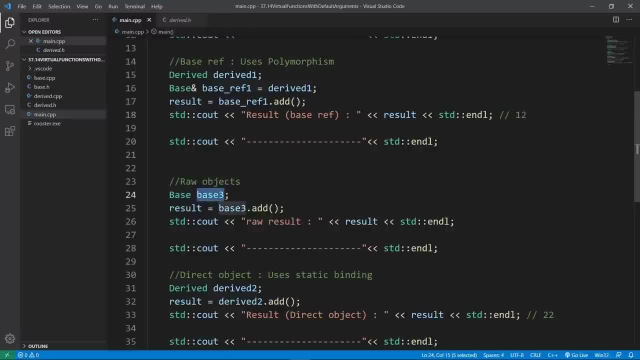 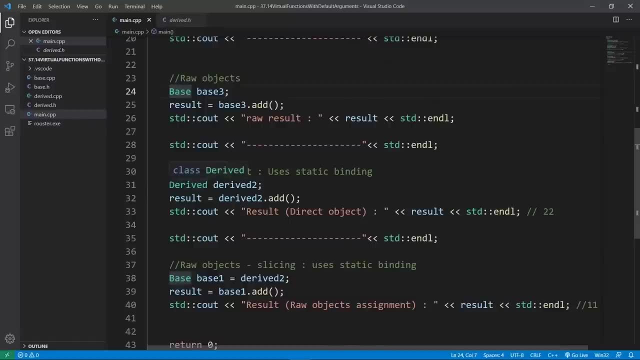 to see which kind of object do i have here. base 3 is a base, so i am going to use the default parameters from base. down below on line 31, the compiler is going to look and see which kind of object do i have here. the object is derived, so i will plug in the default parameters for derived. 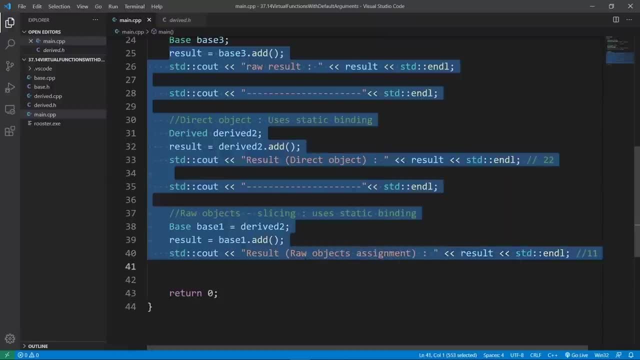 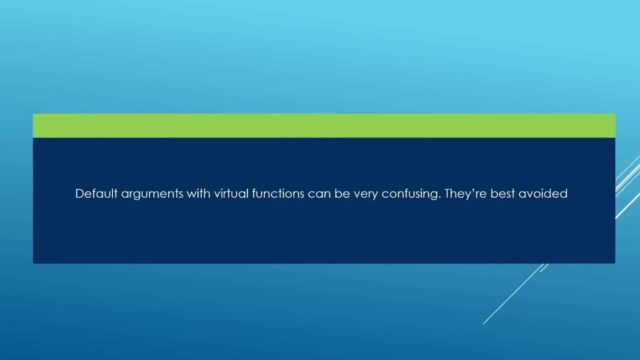 again. this is really what the compiler is going to do with default parameters. the compiler is never going to do dynamic binding and this is going to make your code really confusing again. my advice is to avoid default arguments or devote parameters if you are using polymorphism in your inheritance. 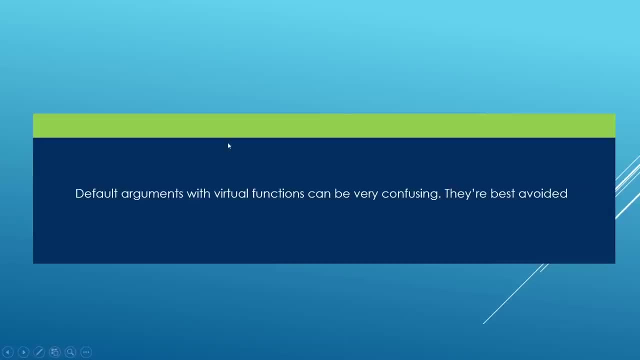 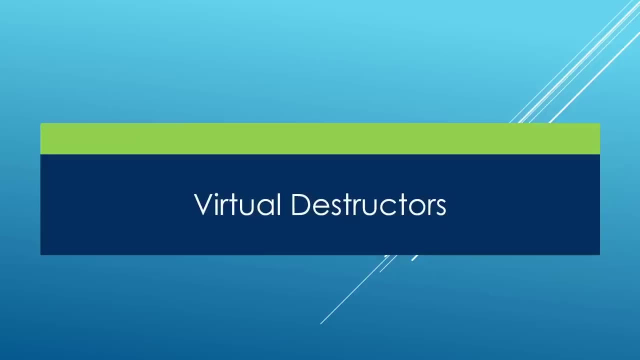 hierarchy. we are going to stop here in this lecture. in the next one we're going to learn about virtual destructors. go ahead and finish up here and meet me there. in this lecture we are going to explore virtual destructors and these are destructor methods you might want to be called using dynamic, binding or polymorphic behavior. 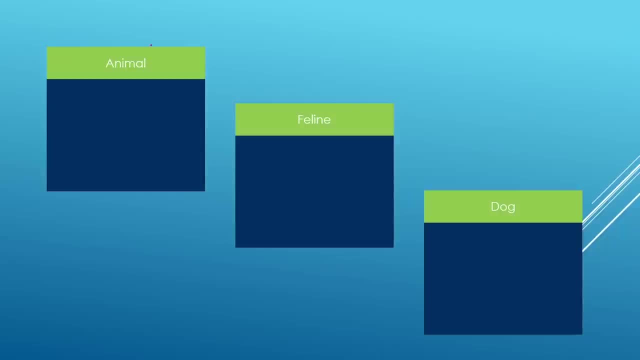 we are going to be using this inheritance hierarchy to play with things. so the animal class is going to be our base class, we are going to derive from that publicly and have a feline class, and we are going to derive from feline and have a dog class. this is the setup we are going. 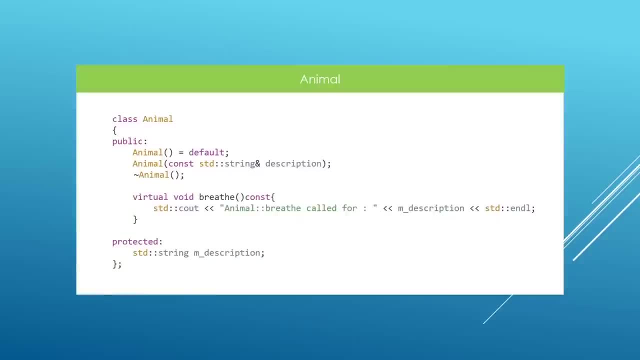 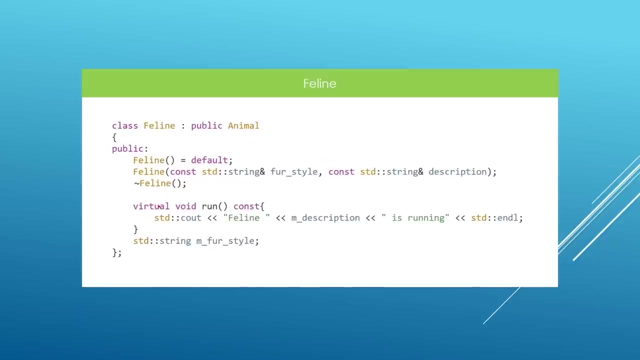 to be using here. now let's look at some code. we are going to set up our animal class like there's nothing really special here. notice that the destructor is a regular destructor we have. we will derive from animal and create a feline class which is going to set up its 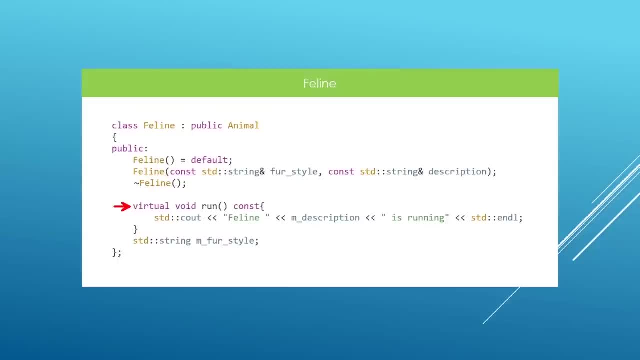 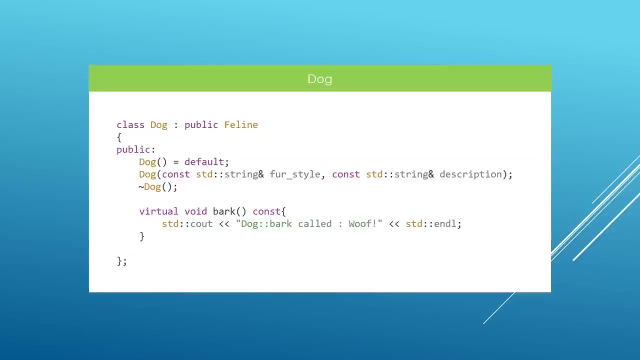 own virtual function which is going to be run. if you want, you can override the breathe method, but we don't want to do that here because we just want to focus on the destructors here and the order in which they are going to be called. we are going to derive from feline and set up 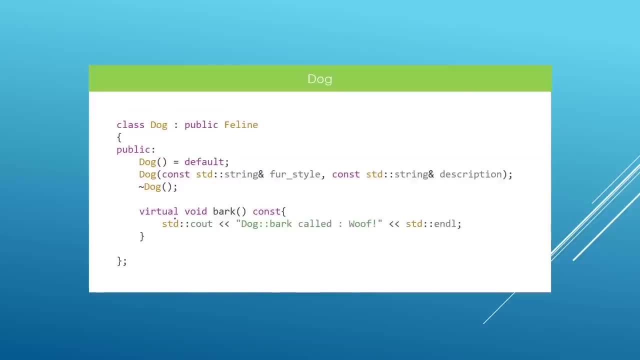 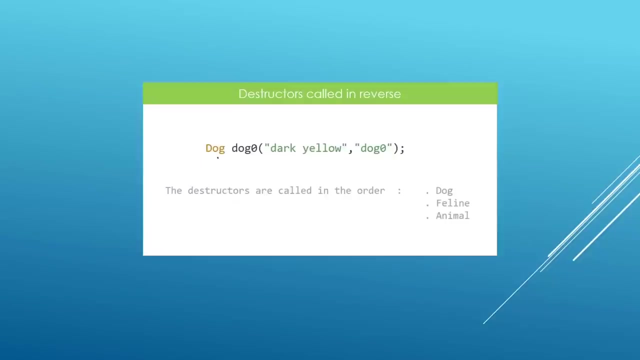 a dog class, and this dog class is going to set up its own virtual function and notice that it has a destructor which is really a regular destructor. now, once we have this inheritance hierarchy set up, we might want to do something like this: we can create a dog object and when it is time for this, 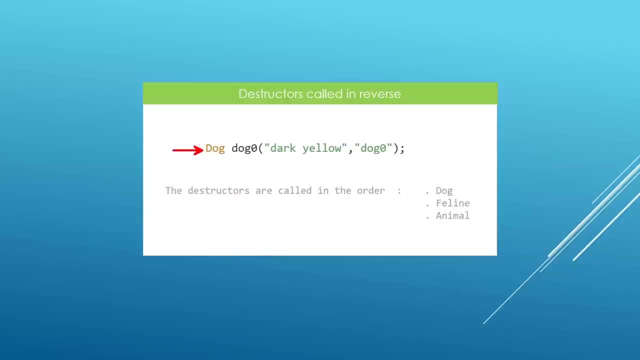 object to be destroyed. i want you to focus on the order in which the destructors are going to be called. we have seen this before: the destructors are going to be called from the specialized to the most base implementation of the destructor, so the destructor for a dog will be called first. 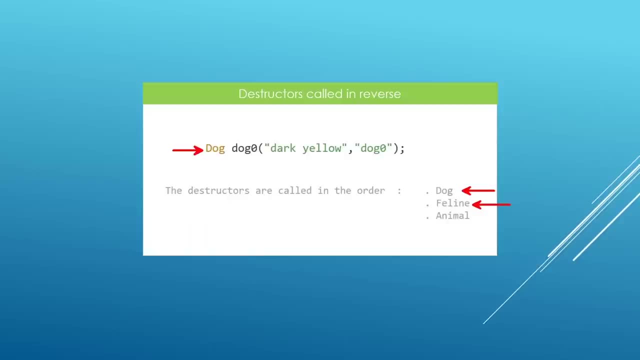 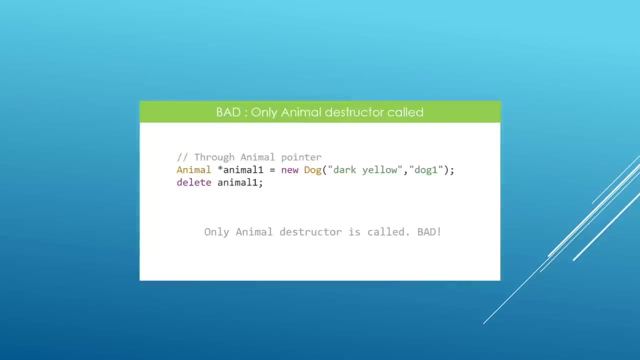 then we will call the destructor for feline, then we will call the destructor for animal. now a problem is going to pop up if we are using a base pointer to manage a derived object with polymorphic behavior that we might want for our inheritance hierarchy here. so we 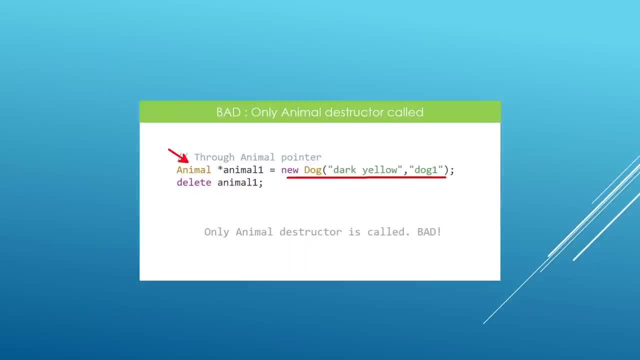 are going to use an animal pointer to manage a dog object like this and when it is time to release the memory for this object, we may be tempted to call the delete operator on our animal pointer here. but this is only going to call the destructor for the base class and hopefully you can see the 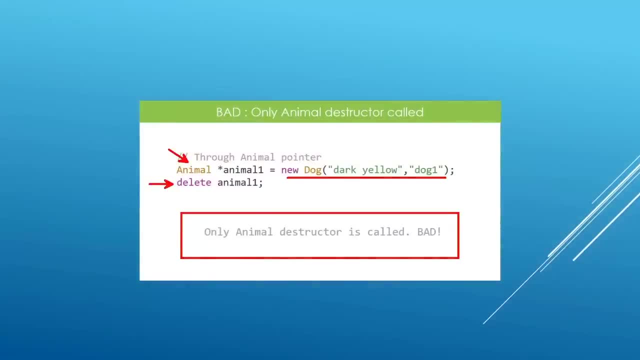 problem here because our destructors are not virtual. the compiler is going to use static binding to decide which destructor to call. so it is going to look at the type of our pointer. it is going to see that it is an animal pointer and it is going to decide to call the destructor for animal here. that's why we get this result. we are 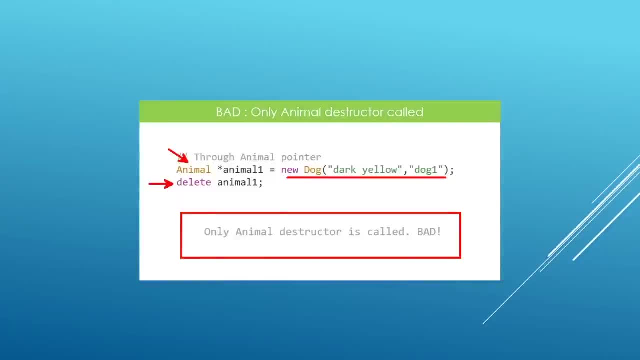 managing an object which is not just an animal. it has derived information in it, but we are only calling the destructor for the base part of this thing. so any piece of dynamic memory we might have allocated in the constructors for feline or dog is going to be leaked out because remember. 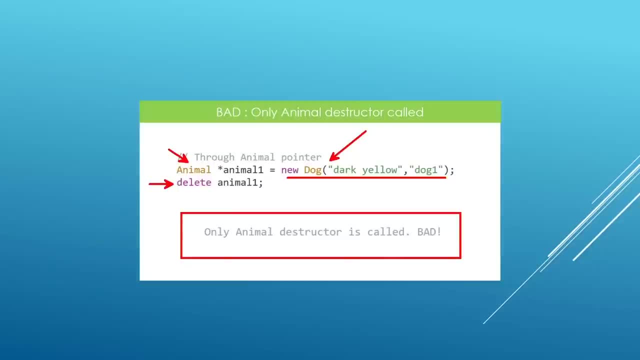 even if we are using a destructor for a dog, we are not going to call the destructor for animal here. if this is a dark object, it is made up of base parts. the foundation for this is going to be animal, and on top of that we are going to build a feline level and on top of that we are going to 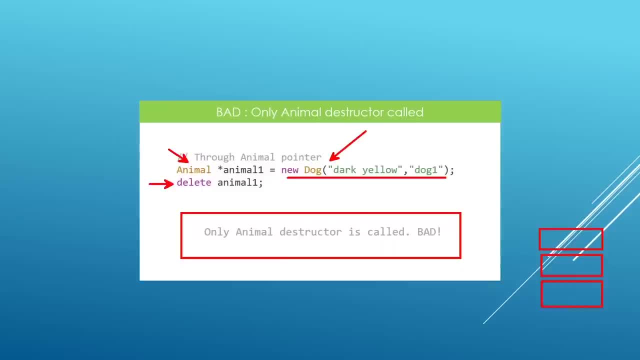 boil. the dog level, in this case only the destructor for doug is going to be called, and any dynamic memory that might have been allocated at the feline and dog level is going to be leaked out, and this is something we don't want. you really need to keep your eye out on this and this also. hard for our animals because their Leben style factory is already a cheeks bald and we are going to have to let our animals do what we don't want them to before we change our stuff case. and anyway, this time we in factということ have had the ability to where we don't have an cảm. 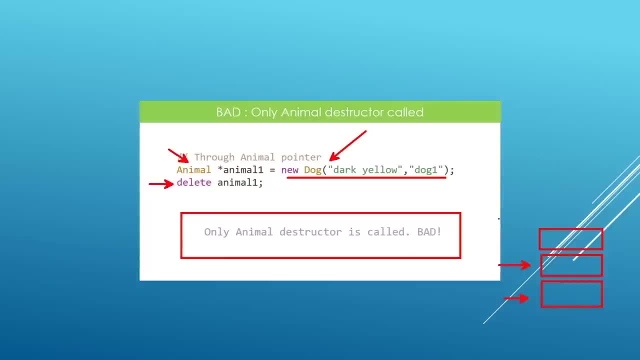 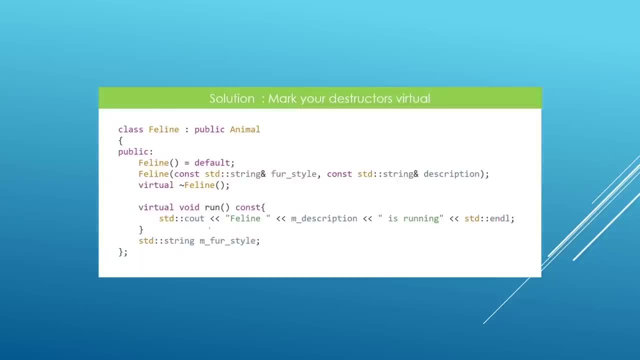 And this is something really bad. you really need to keep your eye out for this. So this is already a big problem, and to solve it we need the destructors to be called, using polymorphism, and you can set that up by marking your destructors as virtual. 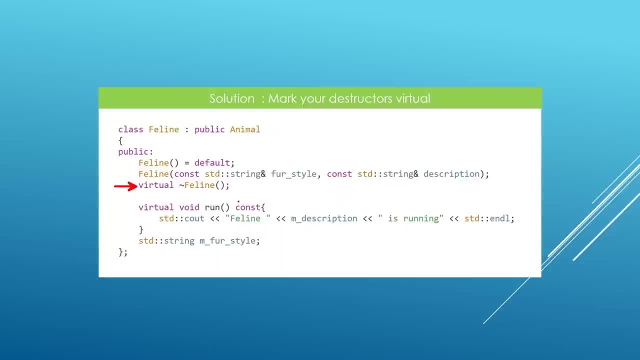 If you do this, the compiler will know that if you are going through a base pointer to manage a derived object, when the time comes for the memory to be released and you release the memory through a base pointer, the compiler is going to call the most specific destructor. 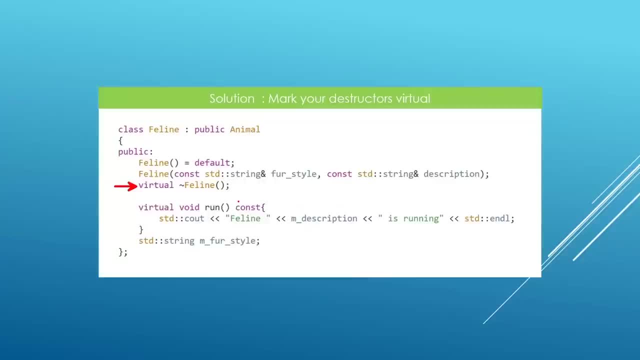 it can find- and this is going to solve our problem- Then we will reuse the order we are familiar with: the most derived destructor will be called and it will call its base destructor, and that's going to happen until we hit the most base class in our inheritance hierarchy and the memory is going to be released exactly. 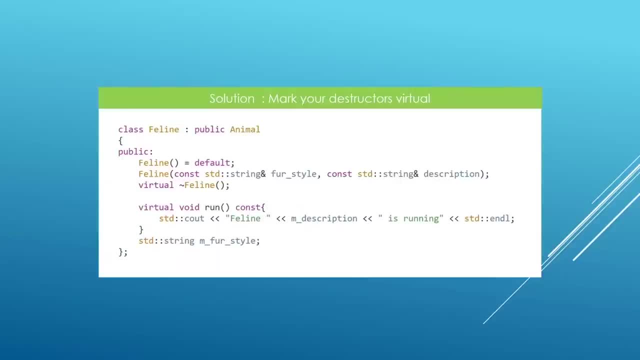 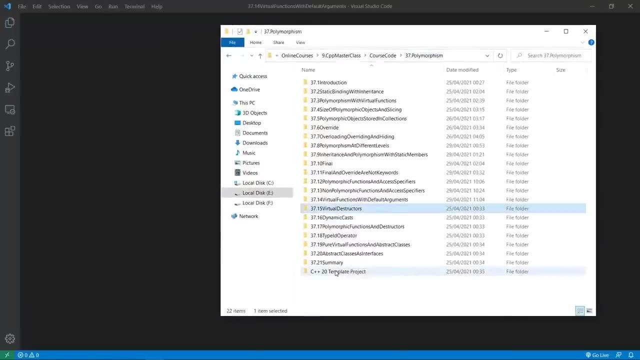 as we would want. Now that you know this, we're going to head over to Visual Studio Code and play with us a little more. So here we are, in our working folder, we are going to learn about virtual destructors, and before we do that, we're going to grab our template files and put them in place. 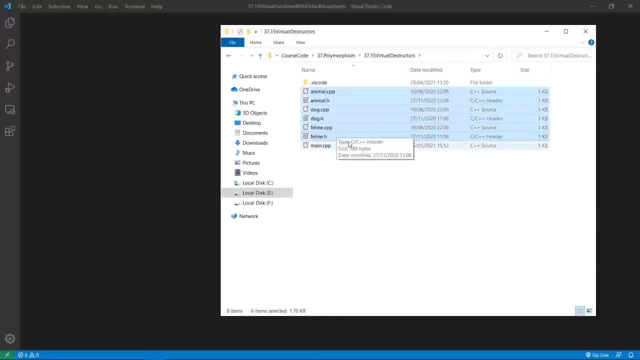 Let's do that And I am going to put in the classes that make up our inheritance hierarchy. our most base class is going to be base. our most base class is going to be animal. After that, we are going to derive from that and create the feline class and we are going 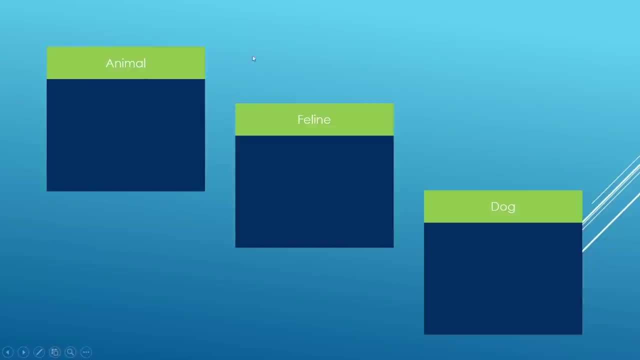 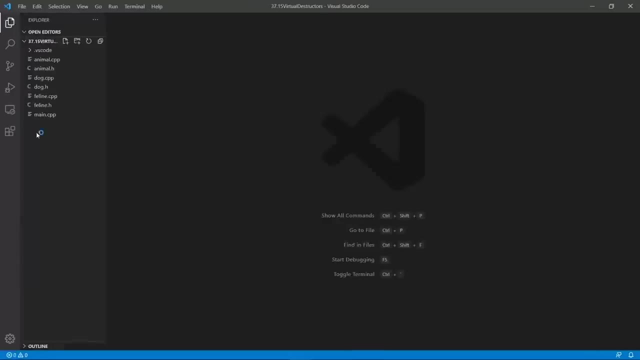 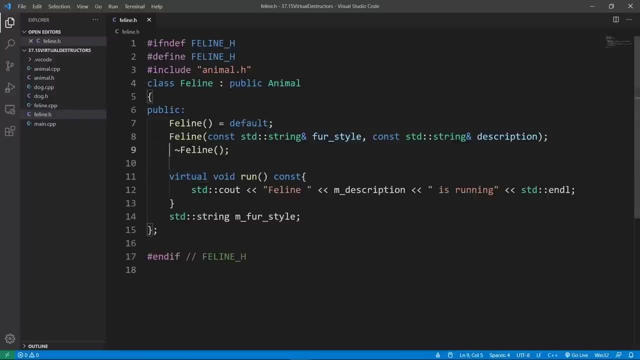 to derive from feline and create a dog class here. This is the inheritance hierarchy we talked about in our slides. Okay, we are going to open this up in Visual Studio Code and this is going to give us our classes here, and we are going to remove this virtual keyword because we want to see what. 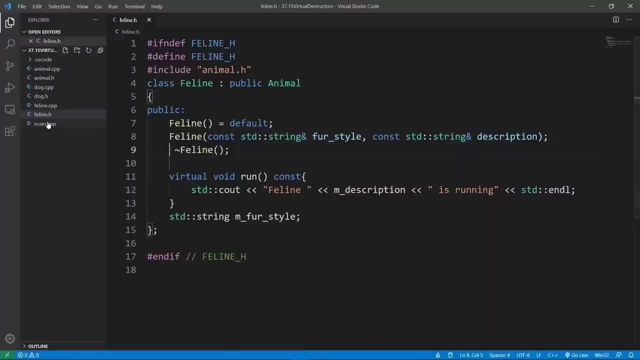 would happen if you don't mark your destructors as virtual. We're going to do that for feline, we're going to do that for dog. let's remove the virtual keyword here. we're going to remove that and we're going to remove that for the animal. 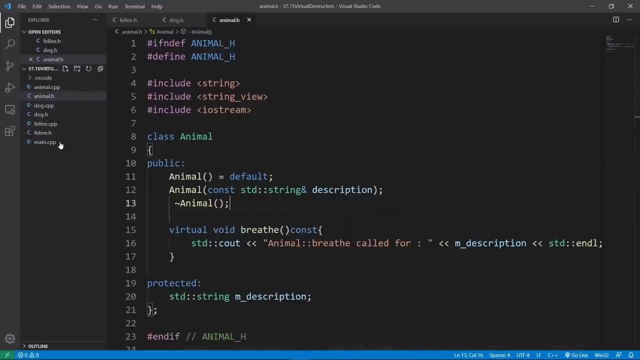 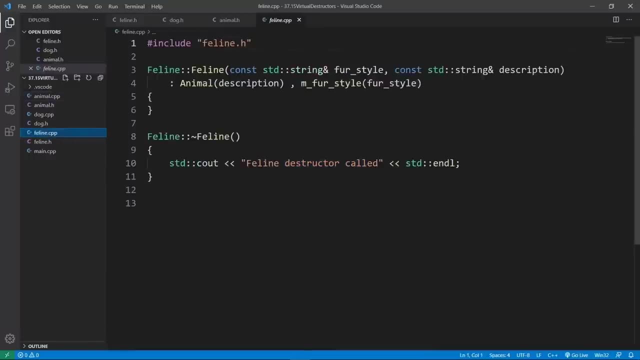 class And we want to see the implementations for our destructors for animal. we are just going to say that the destructor for animal was called for feline. we're going to say the same thing: feline destructor called for dog. we're going to say the same thing. we're going. 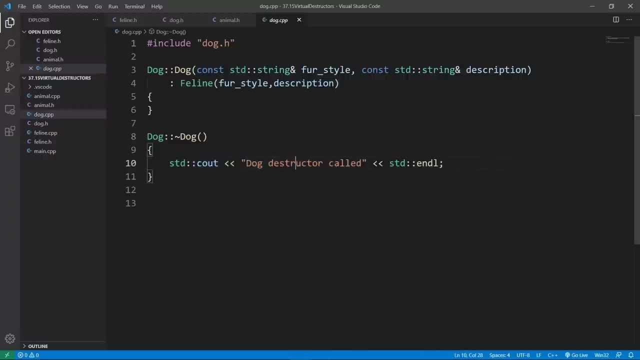 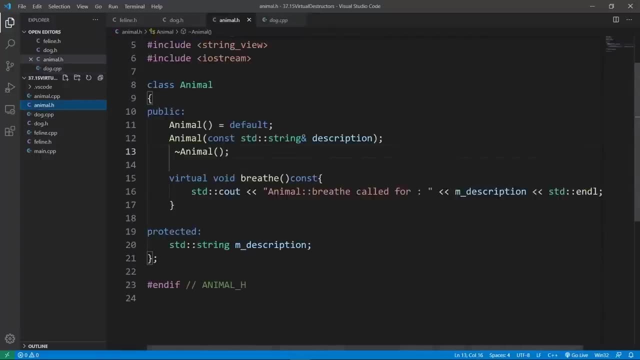 to say: destructor for dog called here. We are using strings as our parameters here, so I think it is a good idea to change these guys to use string view. I am going to do that and come back when this is done. Okay, this is done. 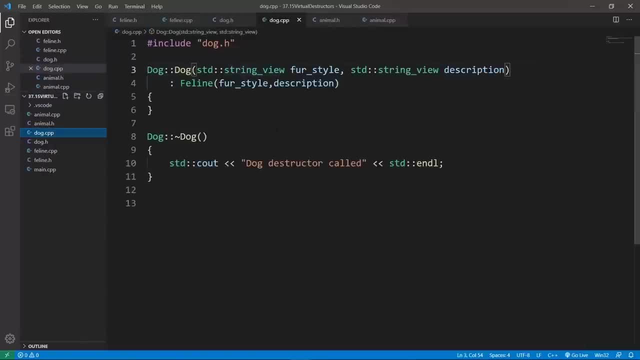 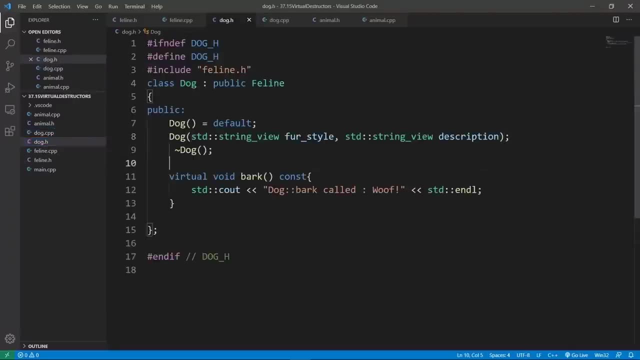 All our parameters are of std string view type and now that we have this inheritance hierarchy, let's make sure none of the destructors is virtual. This is the case here. we can head over to the main cpp file and use this inheritance hierarchy here. 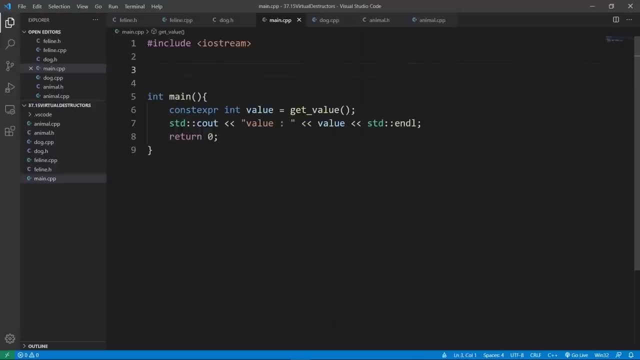 We're going to crack it open and remove whatever we don't need here. We are going to include our dog class, which is going to implicitly include, or its parent classes. so we're going to include dogh here and we are going to create a row dog. 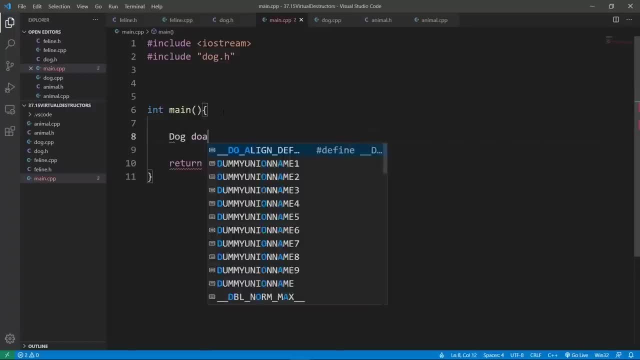 object by default. here we're going to say dog and let's say dog1, we can do that and we might not even give it any parameter. this is going to call the default constructor, and if we go to dog, we're going to see that it is possible to specify information here first. 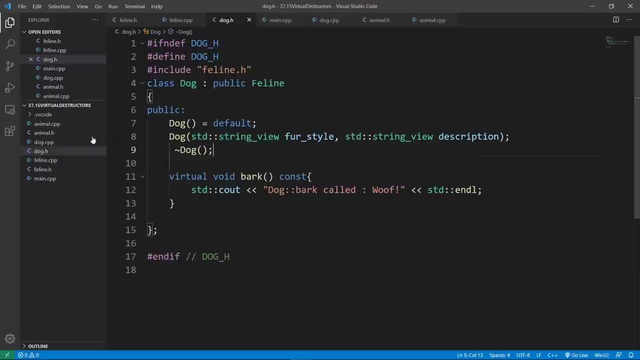 style description. but we're going to ignore this and we just want to see which order in which the destructors are called. Let's build and run this program. we're going to pass this through GCC. the build is going to be good if we clear. let's bring up a powershell window to do that. we're going. 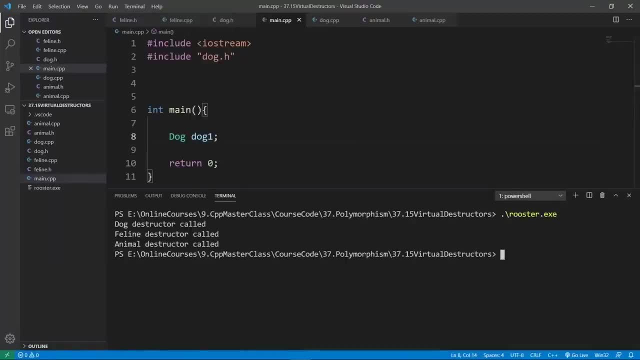 to clear and run rooster. you're going to see that dog destructor was called, feline destructor was called, animal destructor was called, and this is really cool. this is the order we expect by default. But if we don't do something like this and say animal pointer and say p animal to mean, 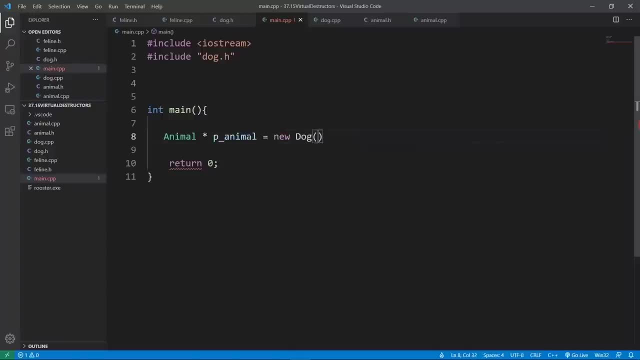 a pointer to animal And we say new dog, we're going to allocate a dog on the heap and we're going to manage that using a base pointer and if we try to release the memory here, let's do that. we're going to say delete p animal. let's see which destructor gets called here. because notice. 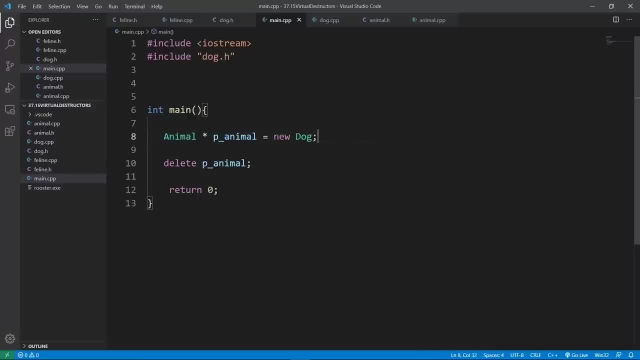 we are using a base pointer to manage a must specific object here, which is a derived class of dog, indirectly, And we will see that we don't get the destructors called In the order that we expect. let's build and run this program to really see this we're. 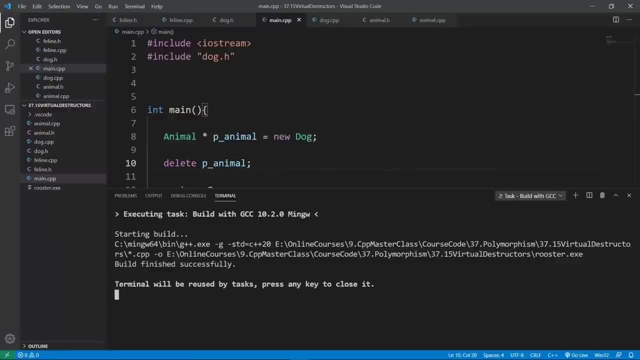 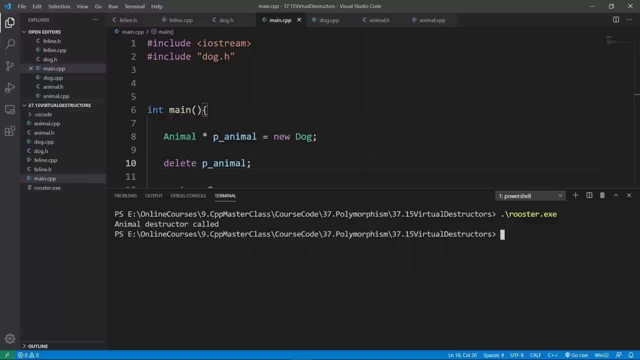 going to use GCC to build it. the build is going to be good. as you see, here we're going to clear and run rooster. now you see that only the destructor for animal is called, even if we are really managing a dog object for things to work really well, we would expect. 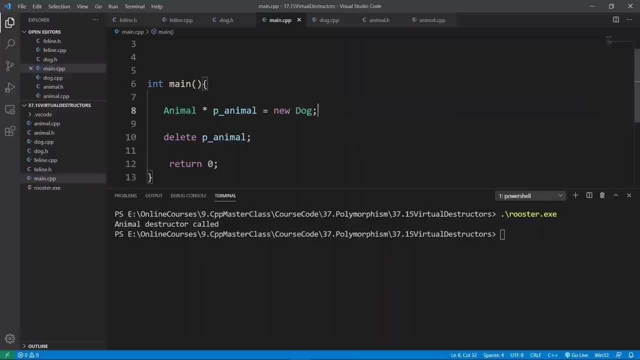 the destructor for dog to be called, and then the destructor for feline and then the destructor for animal. So we're going to use the destructor for animal to release all the memory that might have been allocated by these parent classes for our dog class. If you go back in the CPP file, for example, for each of these classes you're going to. 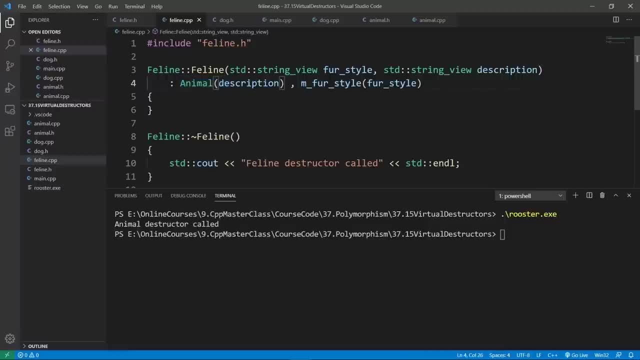 see that the compiler is going to be calling each base class of the current level that we are at In dog CPP. we are going to call the constructor for feline. the constructor for feline is going to be called if it is doing any dynamic memory allocation. we need to release this. 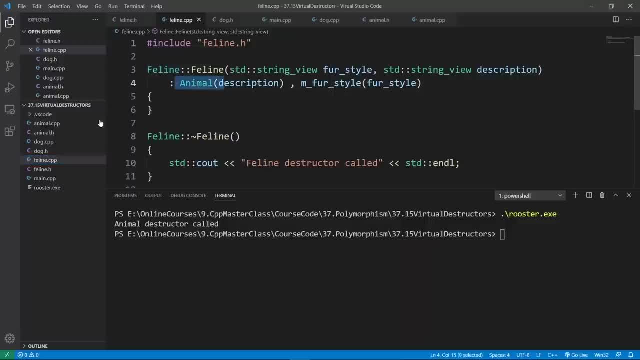 memory Constructor for feline is going to be called if it is doing any dynamic memory allocation and is also going to call the constructor for animal and if animal is doing any dynamic memory allocation, this is going to need to be called. But notice that we are just calling the destructor for animal and if we only call this destructor, 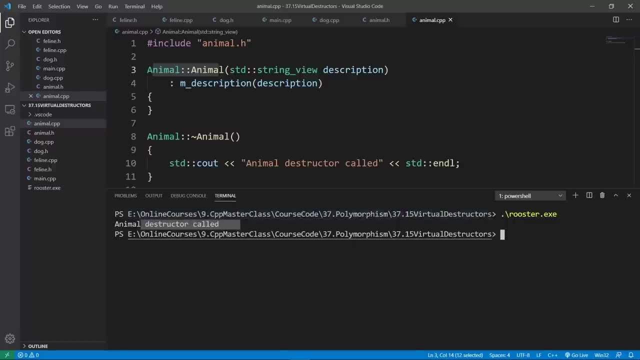 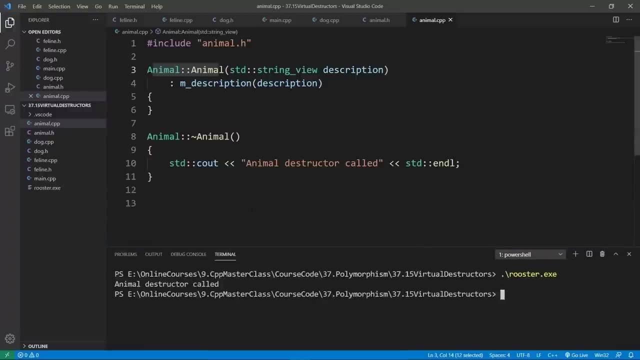 all of the memory that was allocated by the feline constructor is going to be leaked out, because only the animal destructor is going to be called. Hopefully you can see the problem here, But this is not the only problem. the C++ standard says that if you do something like 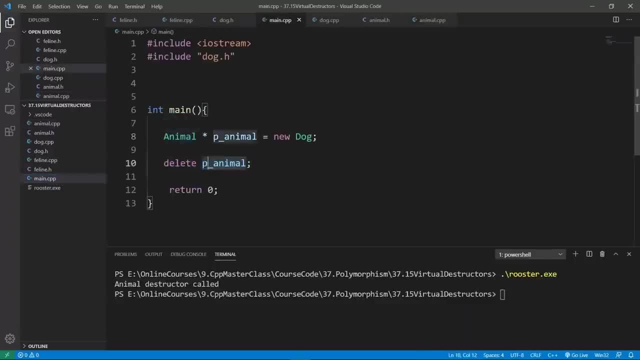 we are doing here And call a destructor using a pointer to the base class, but that pointer happens to be managing a derived object. this is going to give you undefined behavior, So you are not guaranteed to get the same behavior on different compilers on different. 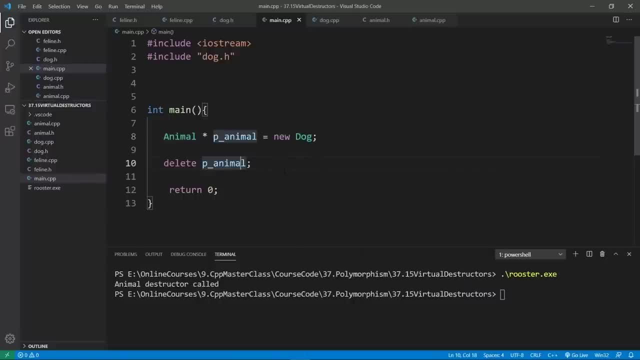 operating systems. So this is something really bad. We want all the destructors in our inheritance hierarchy to be called to properly release the memory that would potentially be dynamically allocated by each level in our constructor. The fix for this is really simple: all you have to do is mark your destructors as virtual. 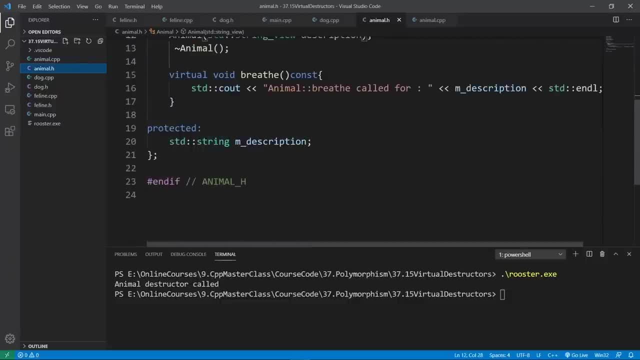 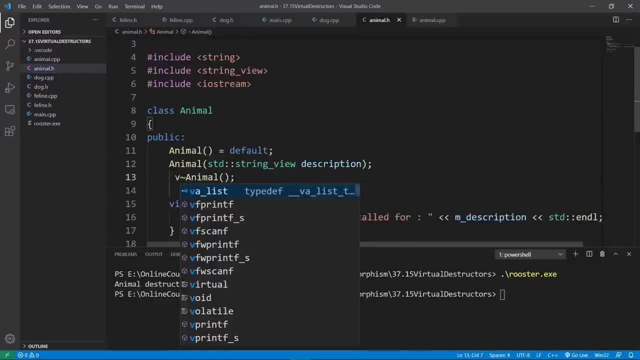 and the compiler will call the most specific destructor for your classes. So all we need to do is go in and mark these guys as virtual. so we are going to do that. The base class destructor is going to be marked as virtual. We are going to go to feline and do the same thing. 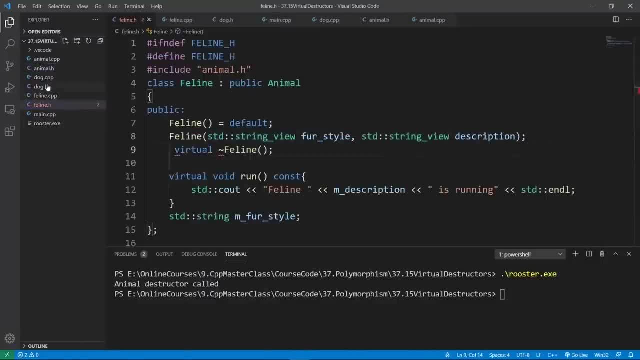 We are going to mark that as virtual and we are going to go to dog and mark its destructor as virtual, virtual. we're going to do something like this and now notice we don't need to change any other thing. if we build our program, we're going to pass it through gcc. it is going to do exactly what we. 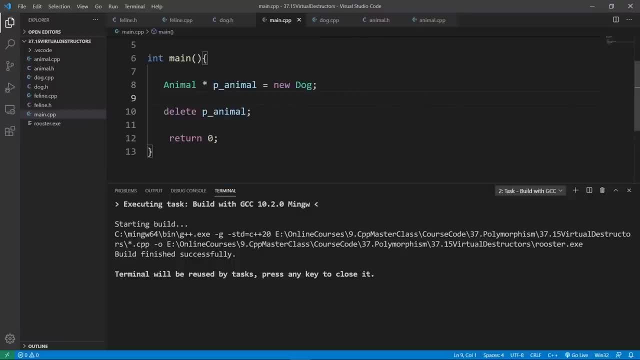 want, because now the compiler will resolve the calls to the destructors polymorphically. because we are going through a base pointer, the compiler will call the most specific implementation for the instructor. because we are going through a base pointer to call the destructor. here the compiler will call the most specialized destructor we can find and it is going to find. 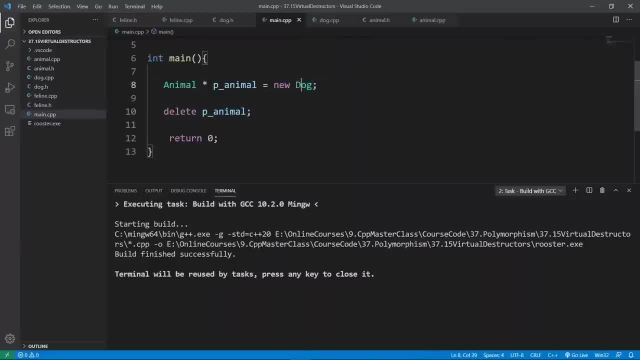 the destructor for dog, which is going to be the most specialized destructor we can find in our inheritance hierarchy. it is going to call the dog destructor, that's going to go the destructor for feline in turn, and then that's going to call the destructor for animal, and our memory is going to 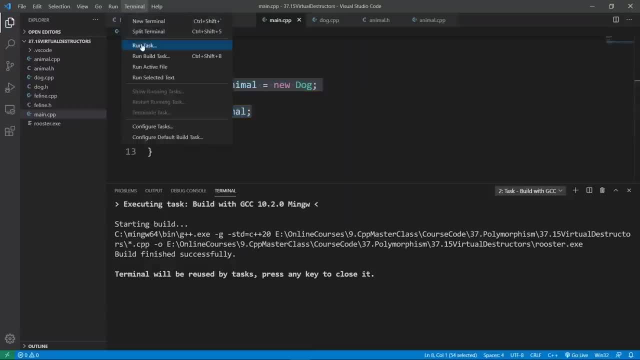 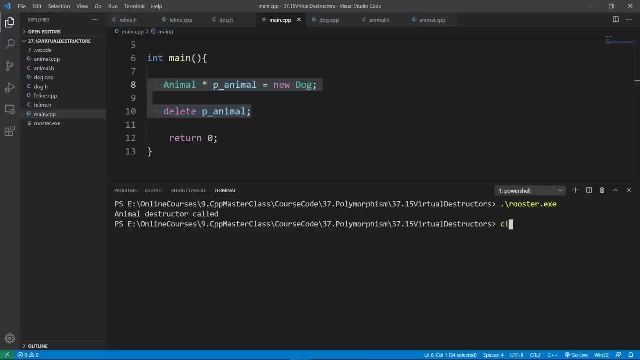 be released properly. that's what we're going to see here. let's make sure we build this again, because- because i'm not sure if i actually built this- the build is going to be good anyway. so we're going to clear and run rooster. now you see that the dog destructor is called, the feline destructor is. 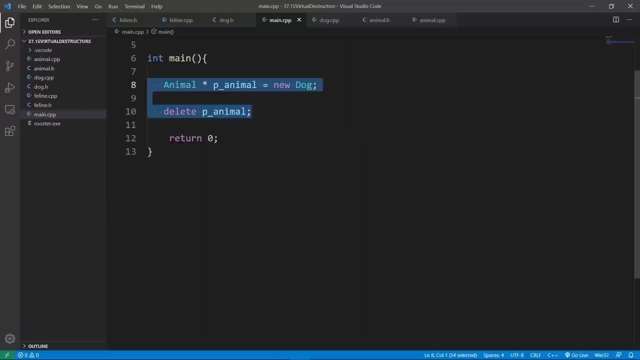 called, the animal destructor is called and everything is just going to fall in place. so my advice: if you are using virtual functions in your inheritance hierarchy, make sure you also mark your destructors as virtual. this is going to save you future headaches you might come in contact with if you are using a base pointer to manage a derived object and you are doing some. 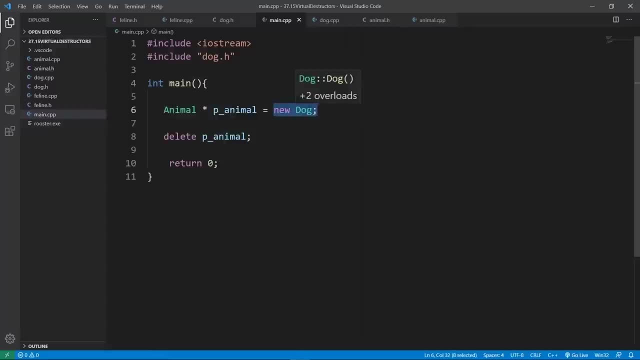 kind of dynamic memory allocations in your constructors, that's going to release the memory properly if you are releasing the memory through a base pointer like we are doing on line 8 here. this is really all i had to share in this lecture. i hope you found it interesting. we are going to 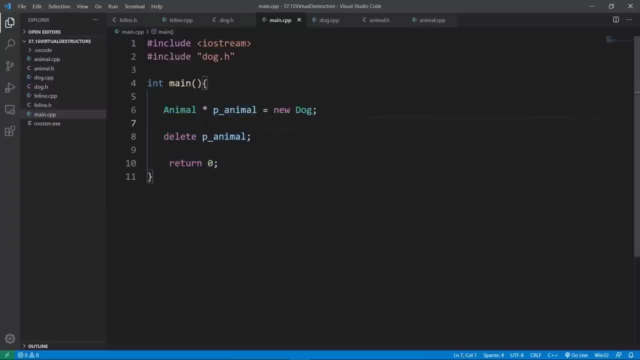 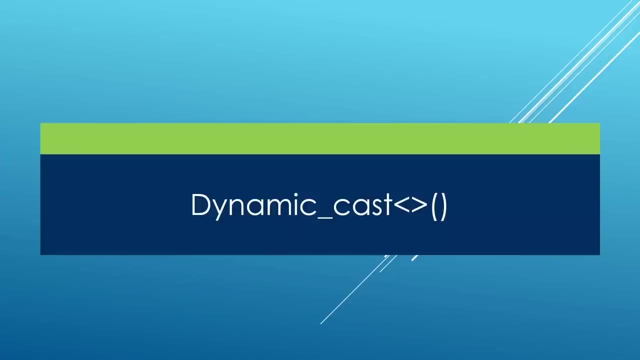 stop here in this one. in the next one we're going to learn about dynamic casts. go ahead and finish up here and meet me there. in this lecture we're going to learn about dynamic casts, and the dynamic casts are a facility we have in c++ to do downstream transformations between our polymorphic types. so if we have a base, 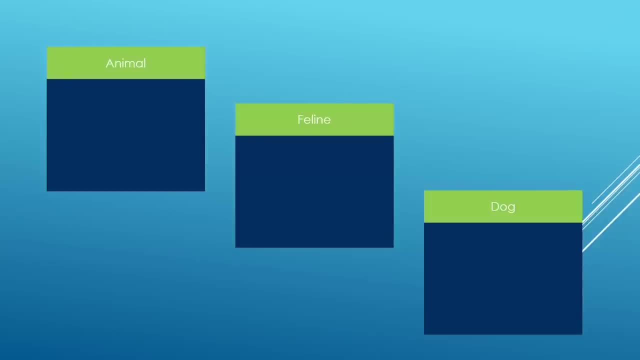 pointer, for example. we can transform it to a derived type and be able to use it like we use any row object, for example. if we do this kind of transformation, we will be able to call inheritance, and this may come in handy sometimes. this is the hierarchy we will be using: our top. 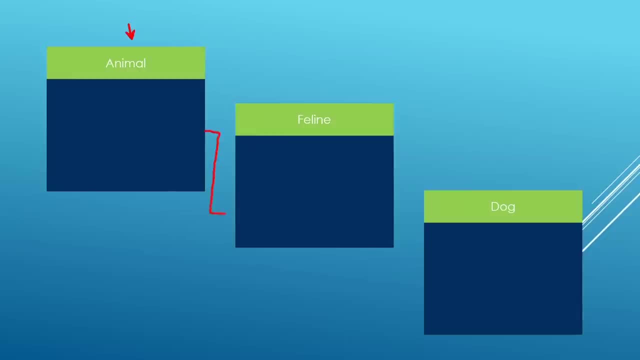 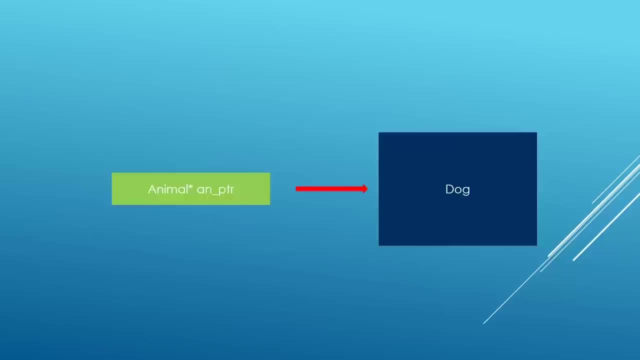 class will be animal here. we will derive from this and create our feline class. and we will derive from feline and create our dog class here, if we have a base pointer pointing to a dog object, for example, the most specialized class we can have in our inheritance hierarchy. sometimes we might want 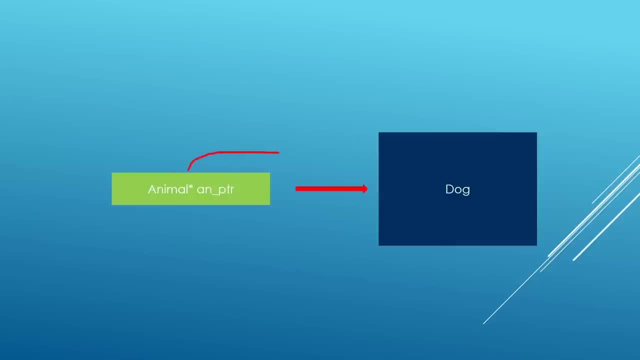 to transform from this base pointer to a derived type and be able to use it like we do in this case. we have a base pointer to the most derived object here and get to the direct most derived object that we can really call anything on, if you remember, with a base pointer like animal here. 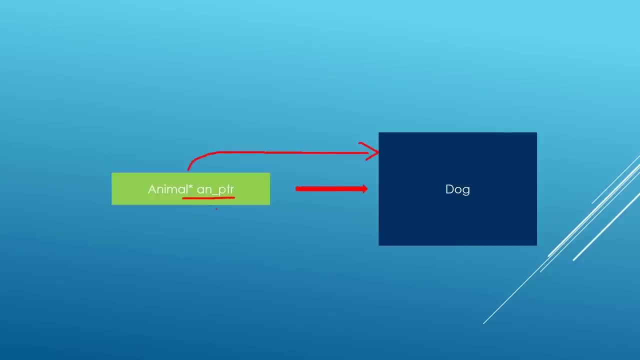 the only thing we can do is really call polymorphic or virtual functions. but sometimes we want to do much more than this. for example, if we want to call non-polymorphic functions, this is not going to work because the base pointer has no knowledge of those functions. so if we need to do that, 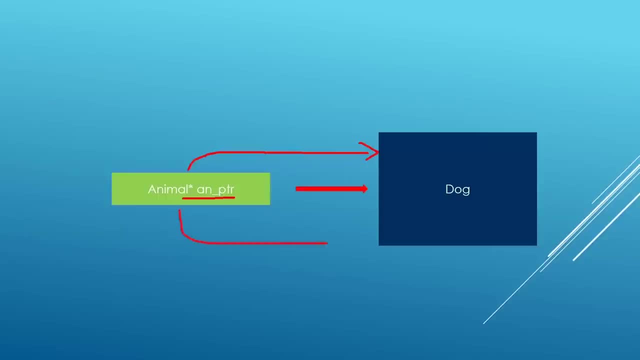 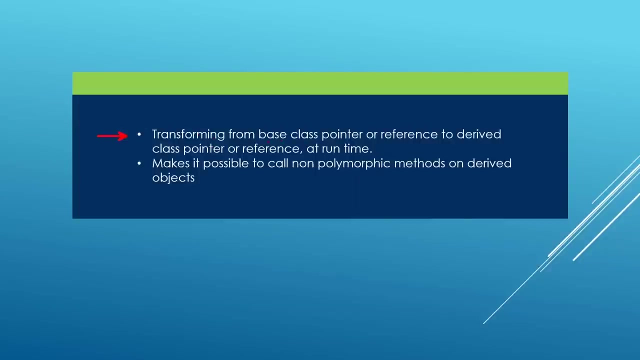 explicitly transforming from a base pointer to a derived pointer is going to give us that capability if the actual object we are pointing at happens to have that method. okay, so this is what we are after in this lecture: we want to be able to transform from a base class pointer. 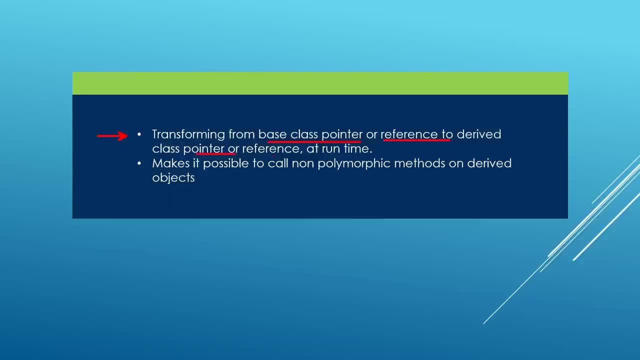 or reference to a derived class pointer or reference at runtime. another way you can take this is to think of the base class pointer or reference as input and we want to get a derived class pointer or reference as output in our c++ program and the main benefit of this. 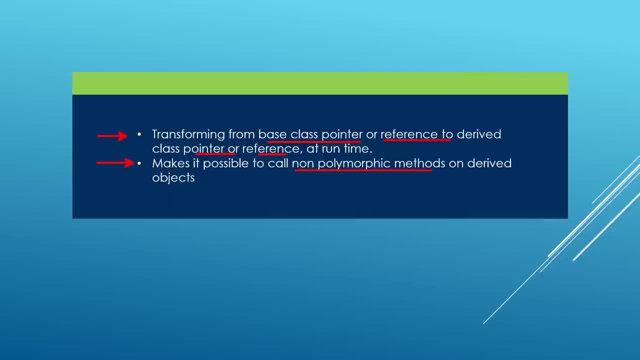 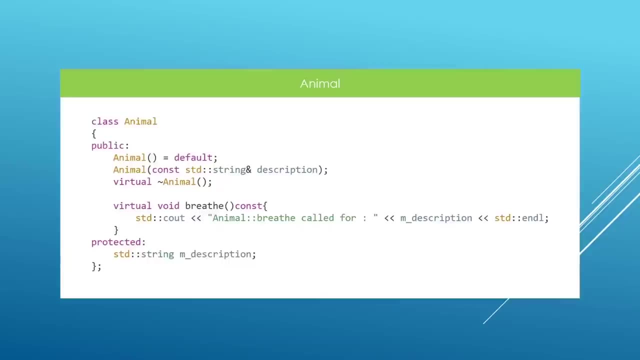 is to be able to call non-polymorphic methods on derived pointers or references. this is going to be super cool in some cases. okay, so let's look at our inheritance hierarchy. here the top class is going to be animal. as you see, here it's going to have a single virtual method. it's going to also. 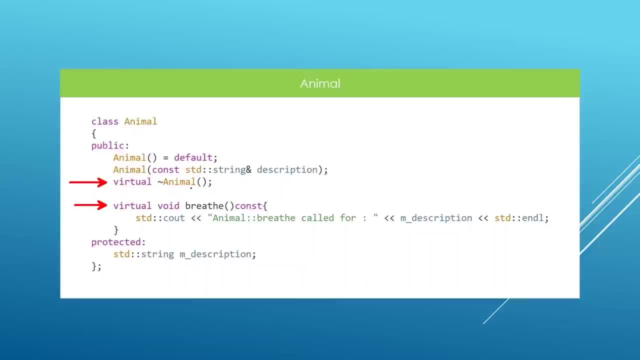 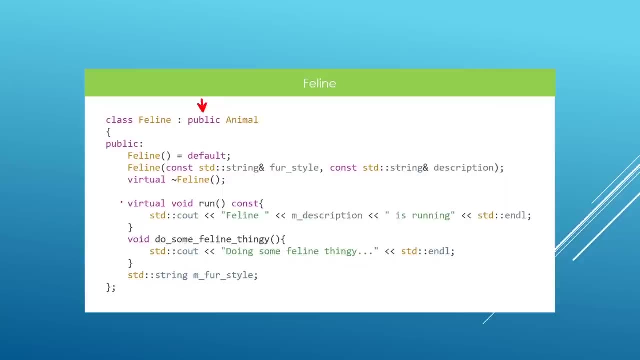 have a virtual disruptor because we know how to do this. now we can derive from this and create our feline class, which is going to be inheriting publicly. it's going to have its own run method and it's going to declare its own other method, which is 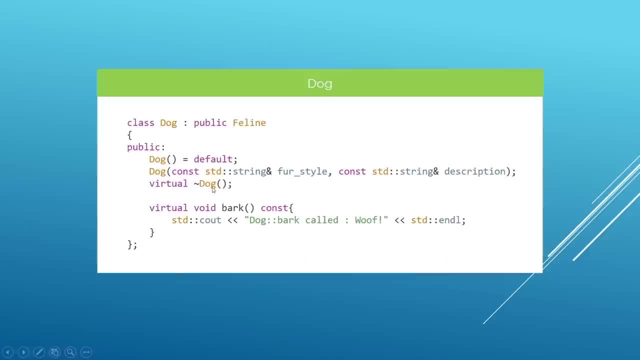 not virtual. we can also derive from feline and create a dog class. this is how we do this, and we're going to set up our own virtual method in dog, which is going to be bark, and we can really do anything we want with this inheritance hierarchy. okay, what we're going to be using as 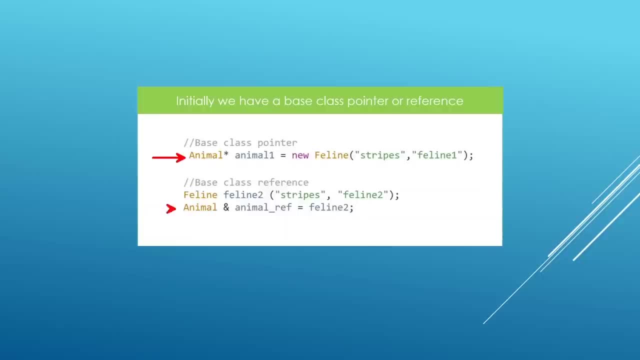 input is a base class pointer or a base-class reference, and we set them up here. this is our base pointer, this is our base reference, and we want to go from these and create a derived class pointer or reference that we can use to even call non-polymorphic functions, and we can achieve that using dynamic casts. 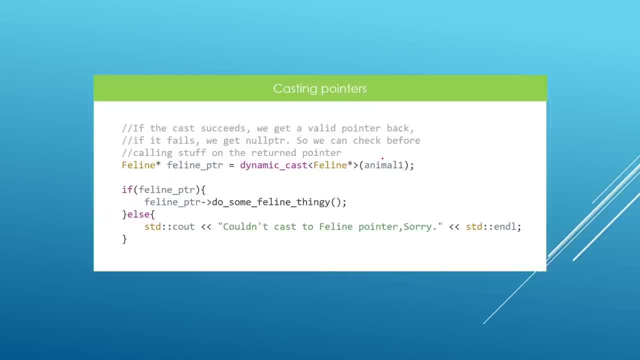 here we're going to show you how you can cast pointers. again, our animal base pointer is going to act as our input and the output is going to be what we want to get out of this transformation, and all we do is say dynamic cast. we specify a. 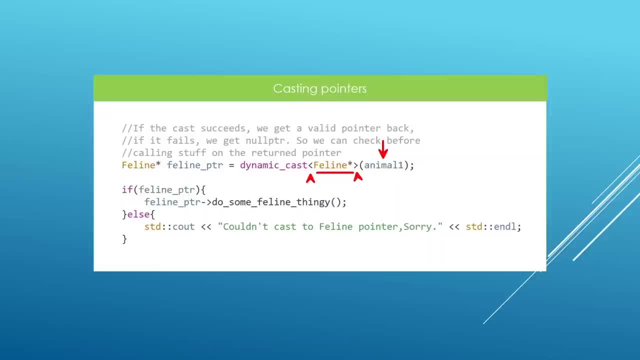 pair of angle brackets inside, we're going to specify the output we want to get and this is usually going to be a derived class pointer. so the base class pointer is going to be within this parenthesis and it's going to be our output and this is going to do the transformation and it's going to give us. 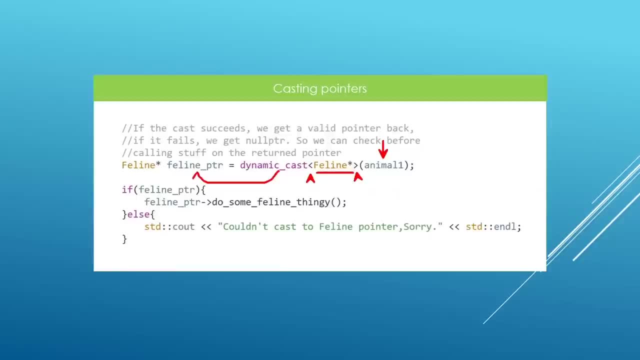 a result that we're going to be storing in our feline pointer here, and if this succeeds, we will have a valid feline pointer here and we can use it to call non polymorphic or non virtual functions, like we are doing here, and this is super. 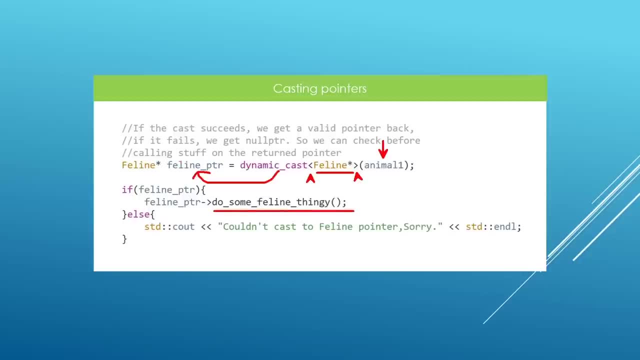 cool. another thing you can do with us is use the result of this transformation in a pointer check, for example. we can check and see if this pointer is not a null pointer. if it's not to know, Szpợyer, we can call our non polymorphic function to. 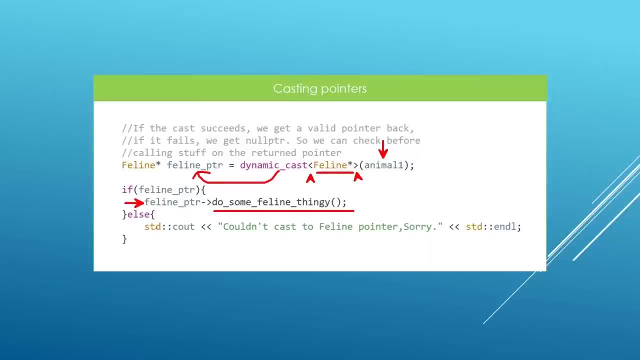 that the result was successful. but if it's null pointer pointer, we're going to fail and fall down here and we can say that we couldn't cast to a feline pointer. and some of you might ask: how can this transformation fail? well, if we go back to our 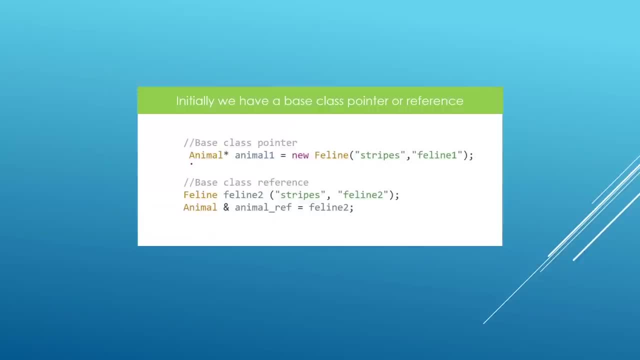 code. here we have an animal base pointer which is really pointing to a feline object in memory. if we try and cast this animal pointer to dog, suppose we want to do this kind of transformation. try to think about this. this is not going to work because we really have no dog information. 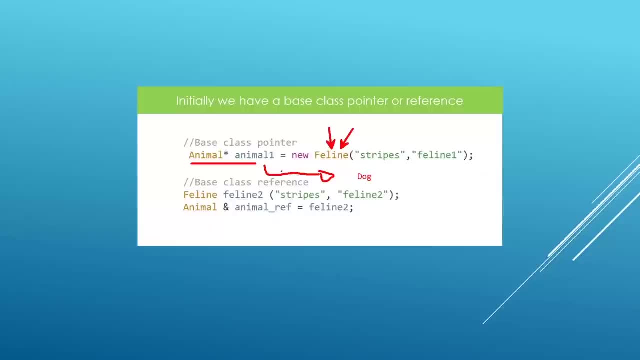 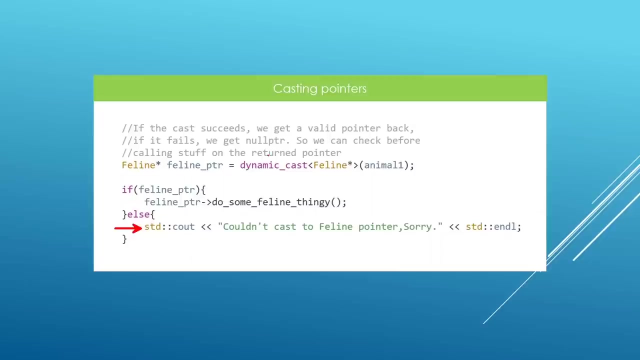 in this feline object and if we try to cast this to dog, the compiler will really have no way to do this and the transformation through dynamic cast will fail and we will say the message here, meaning that we couldn't do the transformation the user asked for. so here we can do the. 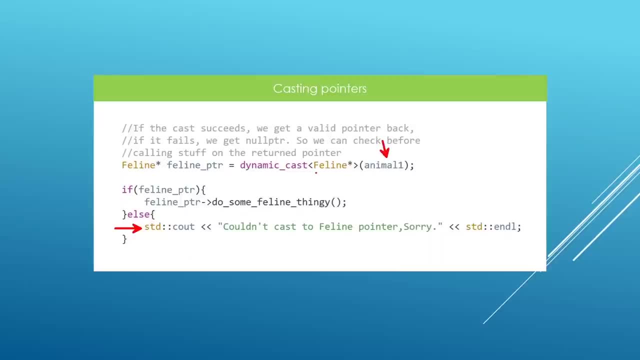 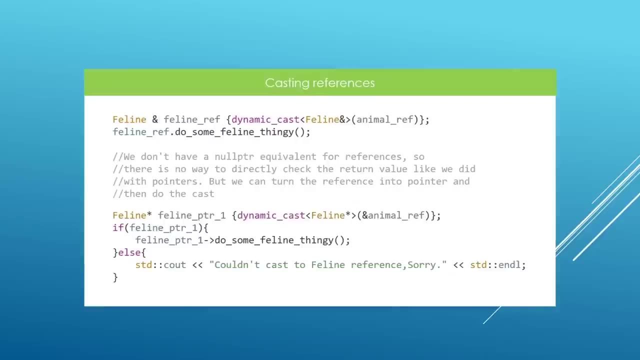 transformation and transform from a base pointer to a derived pointer. but we can also transform to a derived reference and i am going to show you the syntax to do that and it is super simple. we say dynamic cast and we specify our input reference. notice that this is a reference. you. 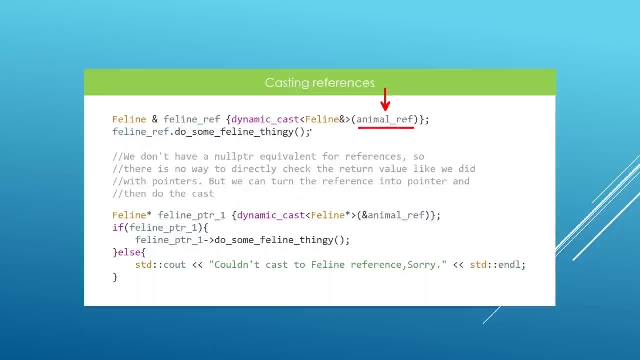 have to put in. it's not a pointer- and you specify the output within this angle, brackets here. once you do this, the output of this is going to be a derived reference and we're going to store this in our feline reference here. once we do this transformation and the 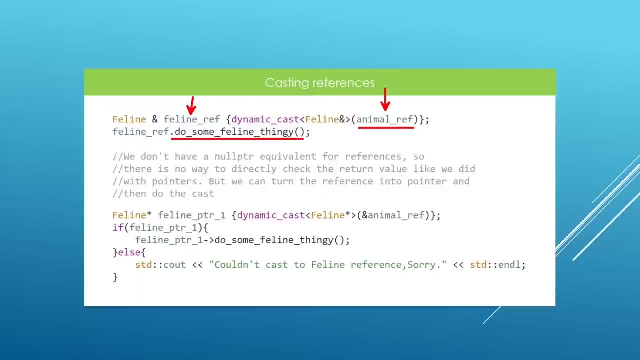 transformation is successful, we're going to be able to call our non-polymer function and this is going to work. but with references. we don't have the luxury to do something like a pointer check, because there is no such thing as a null reference. a reference is always pointed to something and if 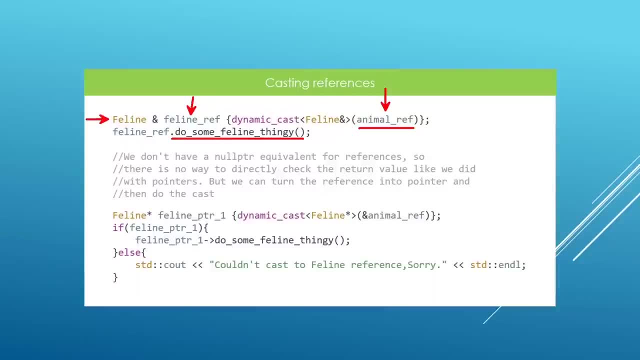 the transformation fails, we will have some kind of invalid reference and if this fails it is probably going to blow up and give us undefined behavior. so you don't really want to do this. i usually don't recommend doing this kind of transformation with references unless you know that the transformation 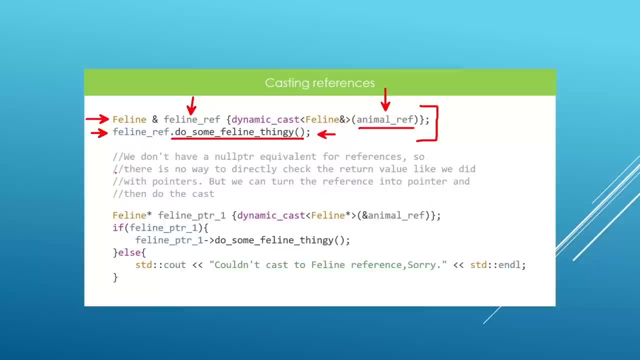 is possible beforehand. what i usually recommend is to pass through pointers, and it is even possible to transform a base reference into a derived pointer, and the syntax to do that is what you see here. okay, and once we do a transformation to a pointer, if the transformation is successful, we're 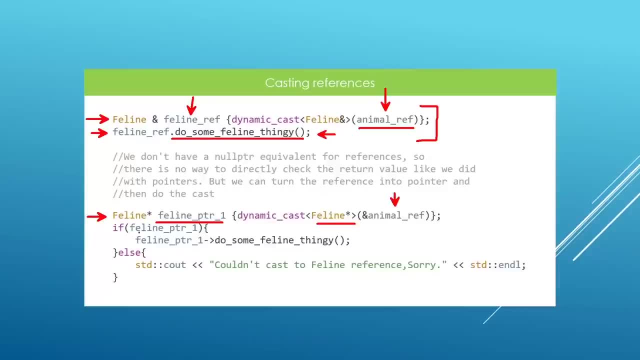 going to have a valid pointer in here. if the fails, we're going to have a null pointer and the check is going to draw us here and we're going to print this message to say that we can't do the transformation here. okay, again, the cast may fail. 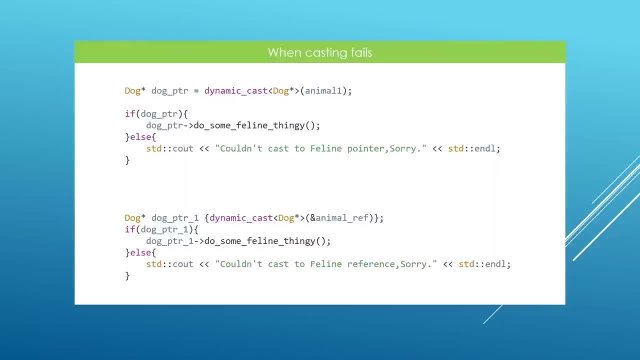 if it fails, while we are trying to transform to a dog pointer, we are going to fall down here and say that the cast failed. we can also do the same thing through references. for example, if we want to transform this base reference to a derived pointer and this fails, we're going to fall here. 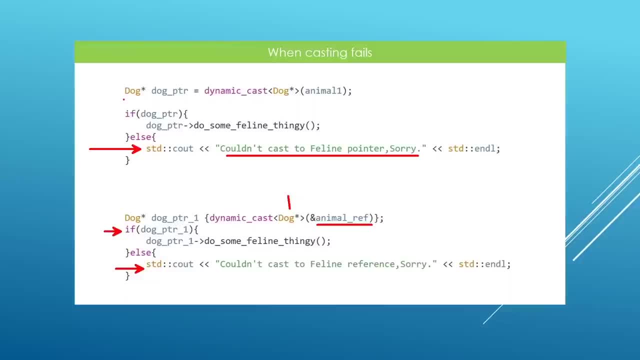 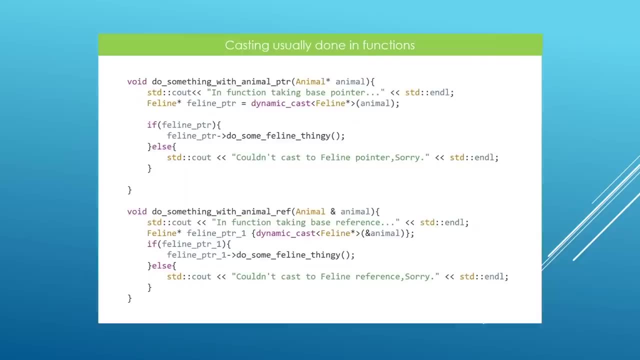 because of the check we are doing here, we can do something like this to make our code much safer to work with. and another thing i should really point out is that in practice, casting like this is usually done in functions where you are passing a base pointer or a base reference as a parameter. 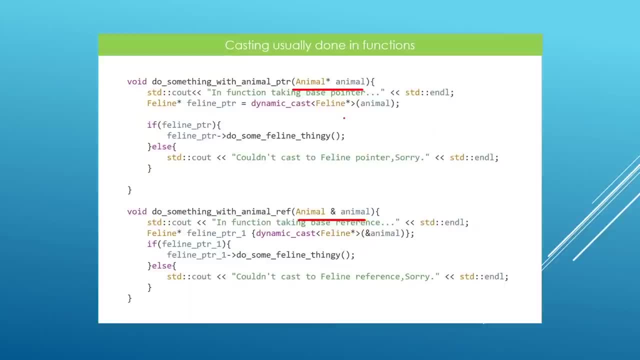 and in this function you somehow need to call a non-polymorphic function. so you might do something like this and take the pointer and turn that into a derived pointer, and if the transformation is successful you're going to call your method, and if this check fails you're going to follow. 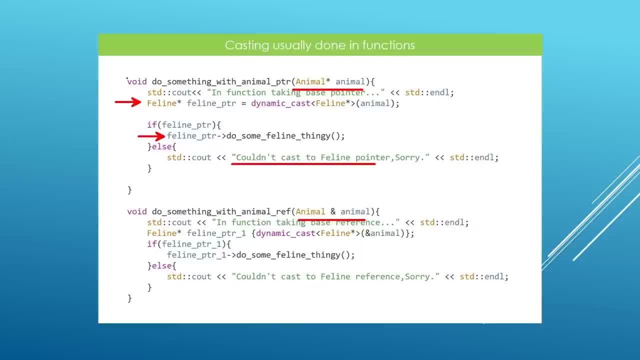 here and print an error message. you can do something like this with pointers, and we can do exactly the same thing with references, but here, because we want to do this check, we're going to transform our base reference into a derived pointer and call our method on the derived. 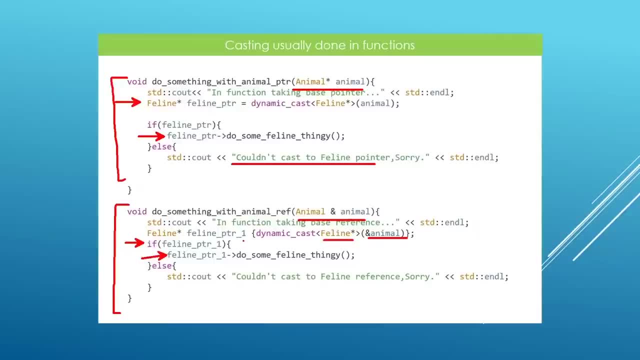 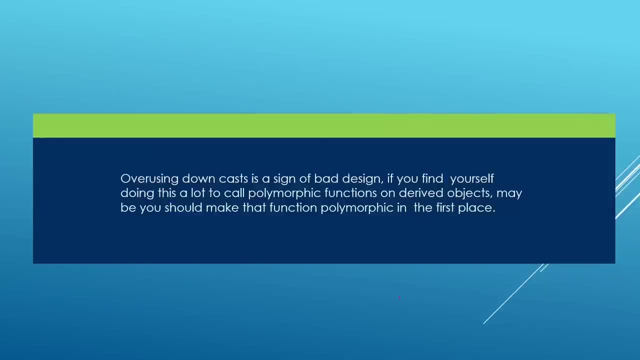 pointer instead. this is going to give us the ability to do this kind of check to make our code much safer to work with a word of caution here: overusing downcasting is a sign of bad design. if you find yourself doing this kind of thing a lot to call non-polymorphic function, that's maybe a sign that you should make that non-polymorphic. 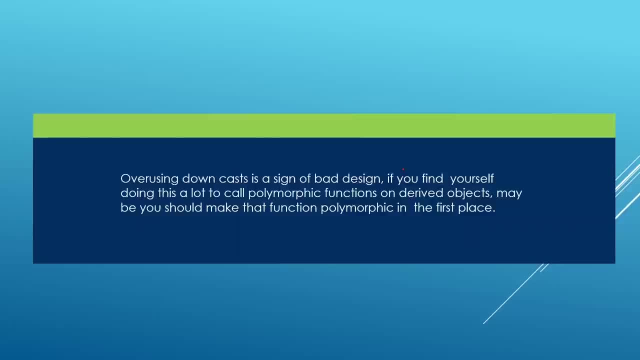 function polymorphic, because that's going to save you from doing this kind of transformations a lot. just make sure you don't overuse this and do it in a few cases where you really need to do this kind of thing. now that you know this, we're going to head over to visual studio: code and play. 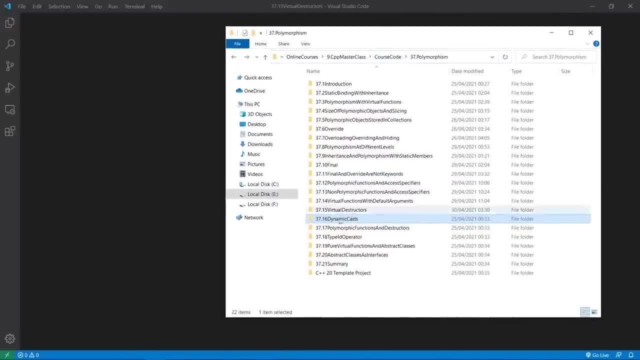 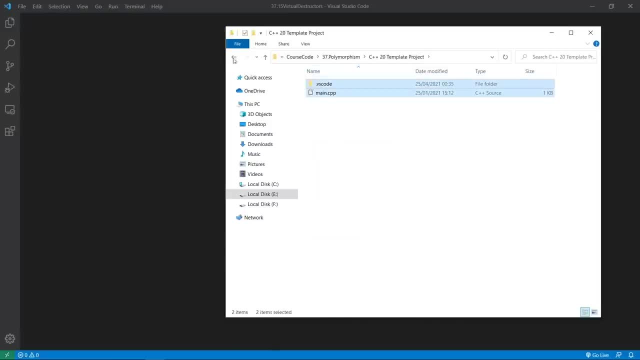 with this a little more. here we are in our working folder. the current project is dynamic casts. we're going to grab our template files and we're going to put them in place. let's do that. and we are going to grab the files that make up our inheritance hierarchy. we're going to put those in. we have animal dog. 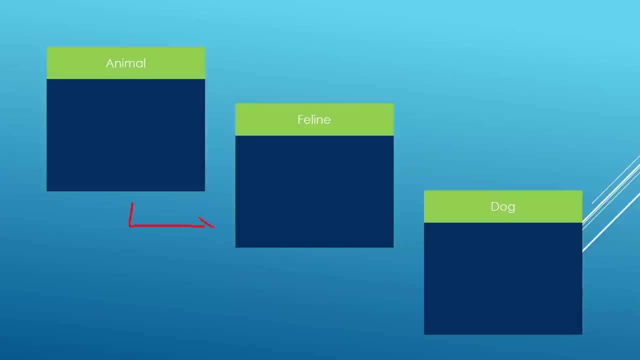 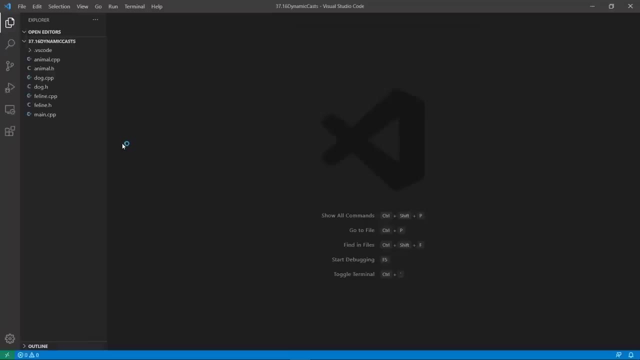 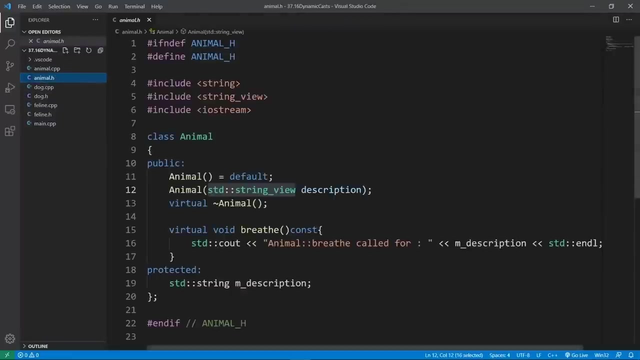 and feline, and this is going to make up our inheritance hierarchy here. once we have this in place, we can open this up in visual studio code by dragging and dropping here and this is going to give us our files. okay, we have our files in here. we can open up the animal class, which is our base class. we 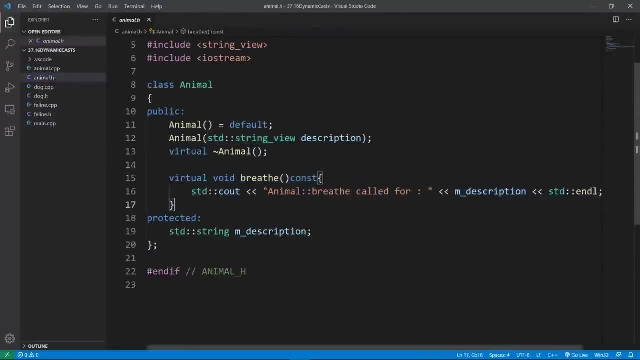 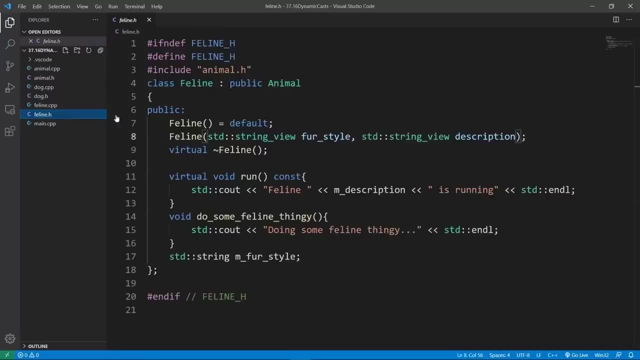 can see that it is really simple. it's just going to have one virtual method, which is breathe. it's going to have a single member variable, which is description. here we can derive from this and create our feline class, which is going to inherit publicly from animal. feline is going to set up its 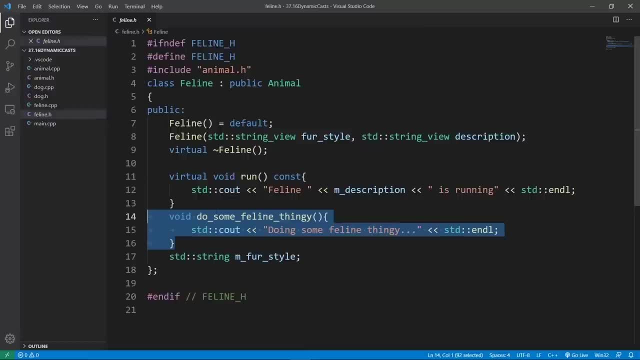 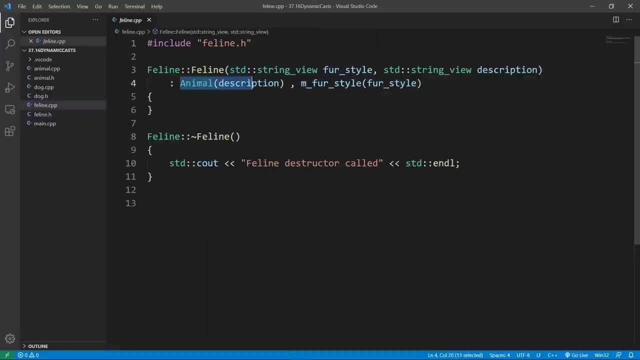 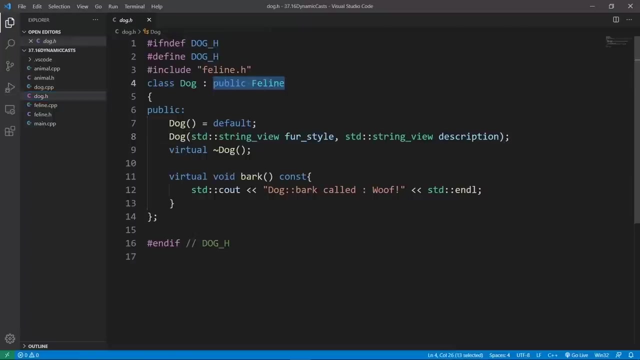 own method which is non-virtual, and we will have a virtual method called run. we can override in downstream class and we're going to have a virtual method called run and we're going to have a virtual destructor which is unAfSense nine virtual method, just in case we're having a work on. 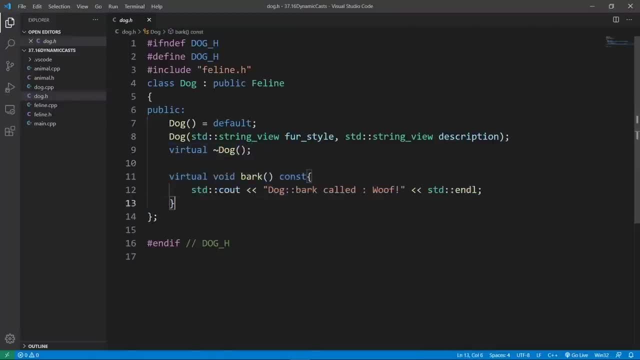 a virtual method which is non-existent. we have the tomato method in our in our inheritance hierarchy, because that's going to make things easier. now we want to go to the main cpp file and play with dynamic casts. we're going to remove whatever it is we don't need here. 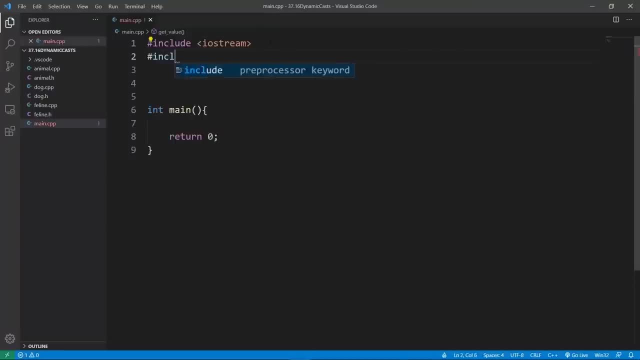 and we can include our most derived class. let's include Doug here. this is going to implicitly include both feline and animal, because this header is going to include its parent and its parent is going to include its own parent. this is the logic. here we are going to start out by using a simple 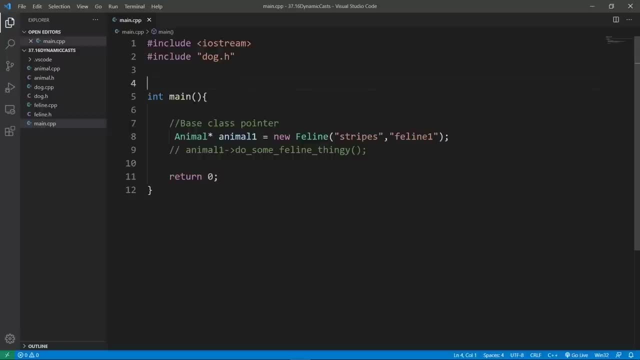 example here and show you that you can't really call non-polymorphic functions from a base pointer that is managing a derived object, and here we have an animal pointer. it is a base pointer and it is managing a real feline object in memory. but if we try and call a non-virtual function through, 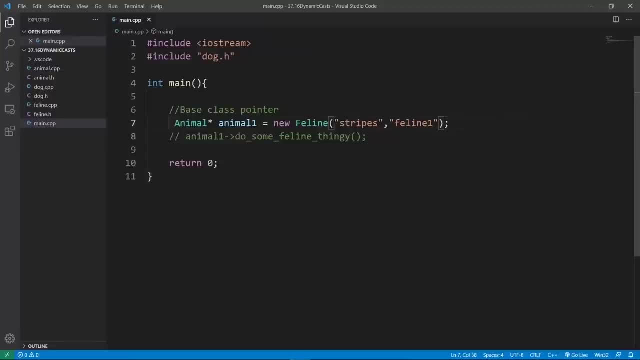 this base pointer. this is going to blow up. this is not going to work because we can't really call a non-polymorphic function through a base pointer, because that's not a virtual function. the requirement to be able to do this is for the function to be virtual and do some feline thingy is not a virtual function. that we know. 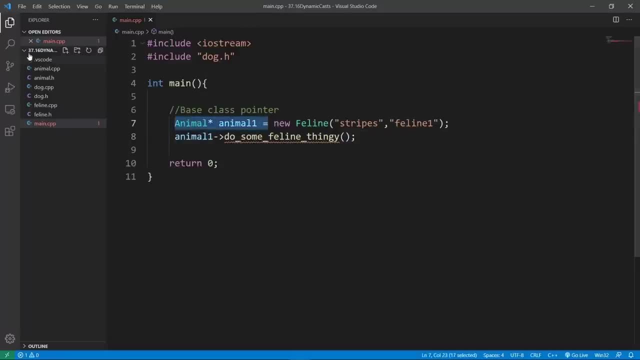 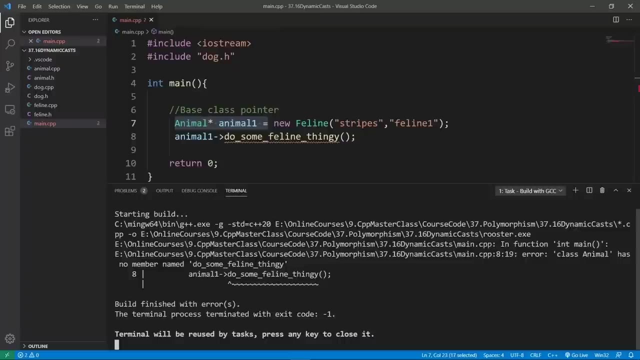 at the base level. so this is not going to work by default and if we try to build code like this, this is going to give us a compiler error. let's pass this through gcc. we're going to do that. we are going to finish the world with errors and if we go up, we're going to find that class animal has no member name to do. 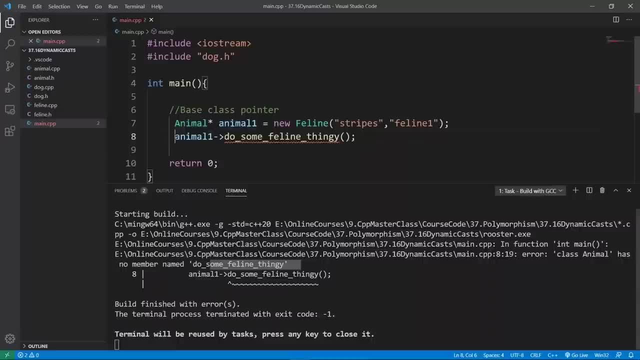 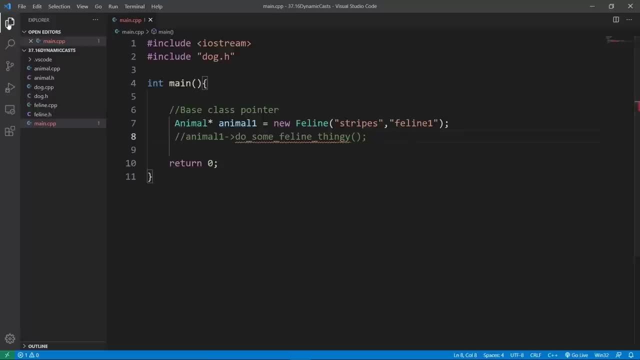 some feline thingy. so this is the compiler error here. this is not going to work. if we need to do something like this, one solution might be to do dynamic casts that we are learning about in this lecture here, and the syntax is ridiculously simple. so we can go down here and put in a 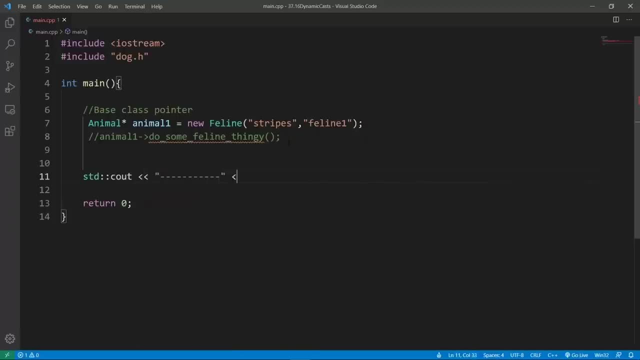 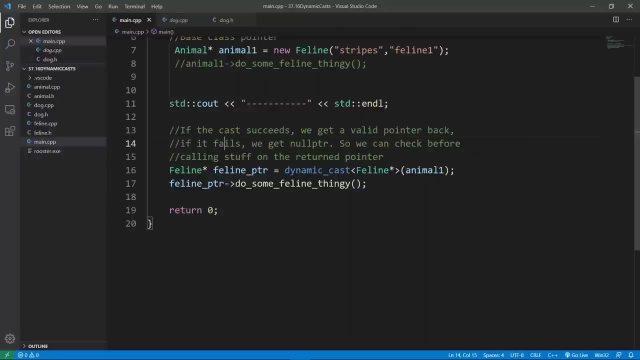 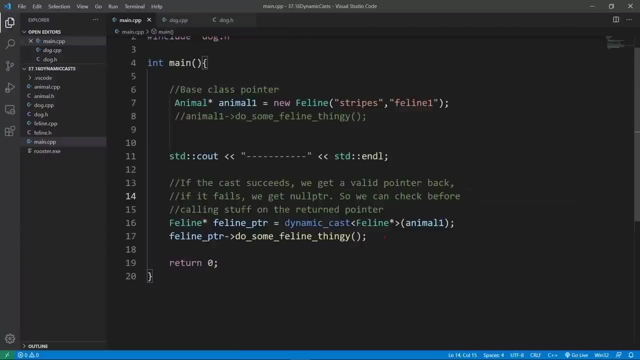 sample separator to be able to follow this lens on our PowerShell window. you can do this if you want, and we're going to do our dynamic cast. for example, if we wanted to do a transformation and transform this to a dog object, this would give us a problem. and let's try and look at this. 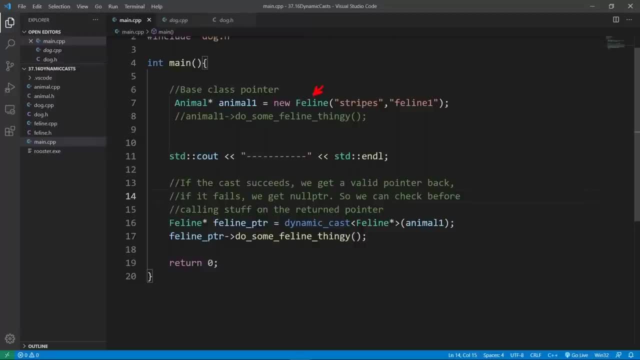 again. we have a feline object here and we are managing this through a base pointer and what we want to do is to take this space pointer and turn it into a dog object. if you look at this, remember that we don't really have any dog information in our feline object. this is going to 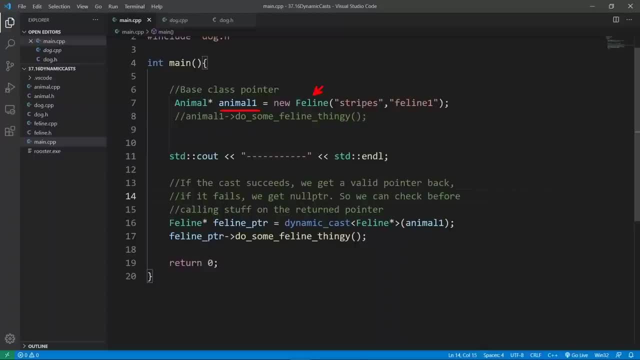 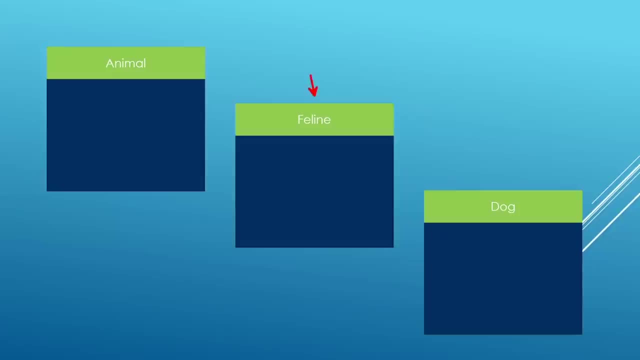 just go up to the level of feline, but we want to transform this to a dog. to make this super clear, let's look at our inheritance hierarchy again. what we have is a feline object and the information we have really goes up to this level, and we are managing our feline object through a base pointer. 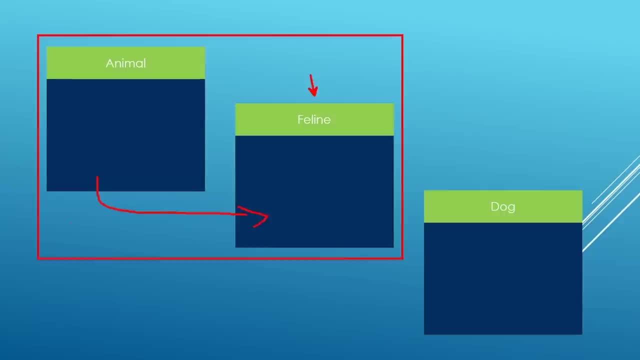 this is the setup we have, but we want to do the transformation and turn this base pointer into a dog object and this is going to blow up, especially if we have any dog specific member variables. this is going to blow up. this is not going to work if we try to access dog. 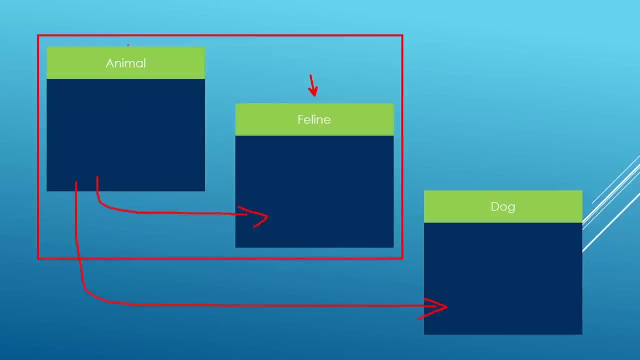 information through what we get through the transformation to animal, to dog, we're going to get a crash because we have no such information and we're going to look at a simple example to really drive this home. so what we're going to do is go back to our dog class and we're going 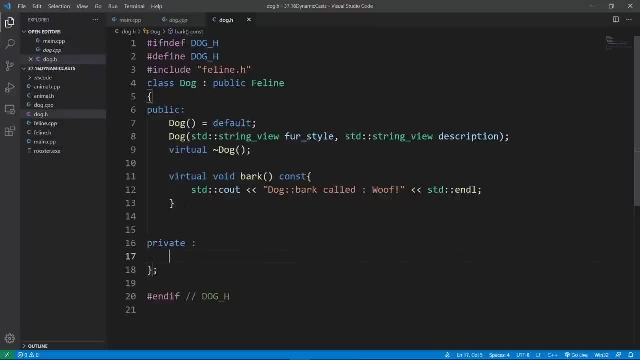 to put in a simple member variable. we're going to make it private and, for example, we can make this a member variable to keep track of the speed for the dog. we can do this and we're going to initialize this to zero by default and we're going to set up a function. 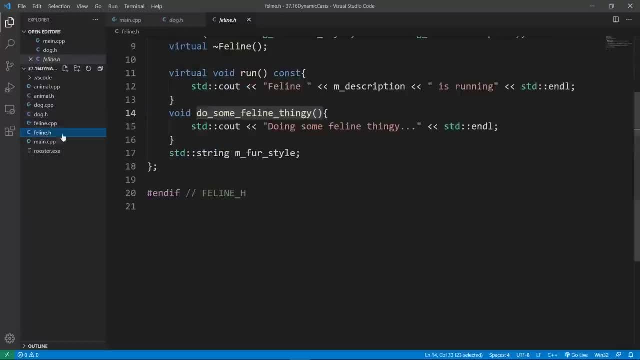 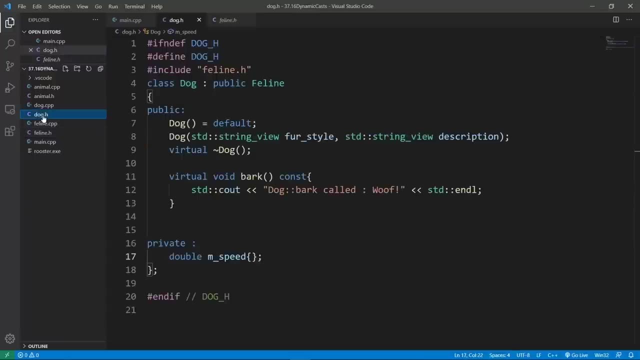 which is going to print some dog information. let's go back to feline and copy the do some feline thinking method and we're going to do some dog thingy. that's what we're going to do here. I am going to put in this method and adapt it a little bit. we're going to do some dog thingy and we're 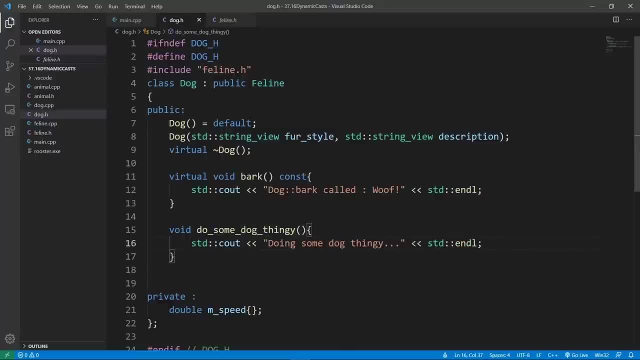 going to account for that in the body. but we also want to print the speed for this dog here. so we're going to say speed and we're going to this out. suppose we have this kind of setup in our inheritance hierarchy. here a dog object has some dog specific information. it has an additional member variable which is m speed. here we won't. 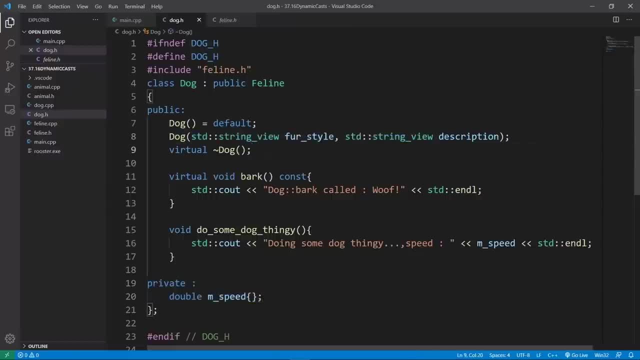 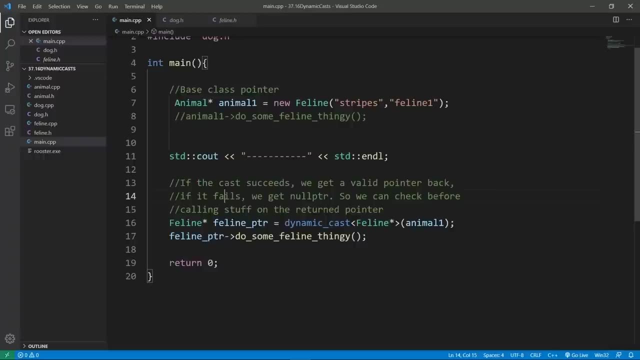 worry about initializing this from the constructor. you can do that if you want. all we really want is to add some extra data at the dog level and we're going to see that if we try to transform to dog, this is going to give us a few problems. so what we want is to turn this animal base pointer. 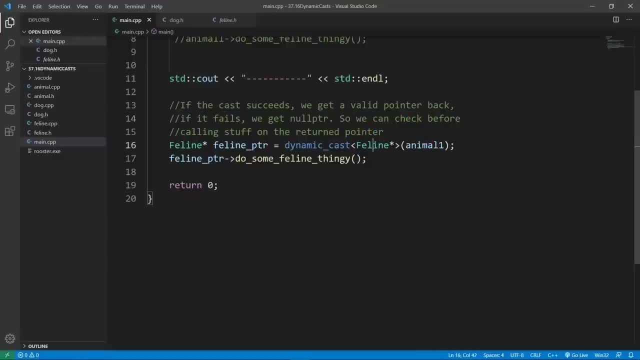 into a dog object. let's do this. we're going to change this to dog and the resort object we get is going to be a dog pointer and we want to call the do some dog thingy method on the pointer we get as a result of this transformation here. let's see what happens. you're going to see that this is. 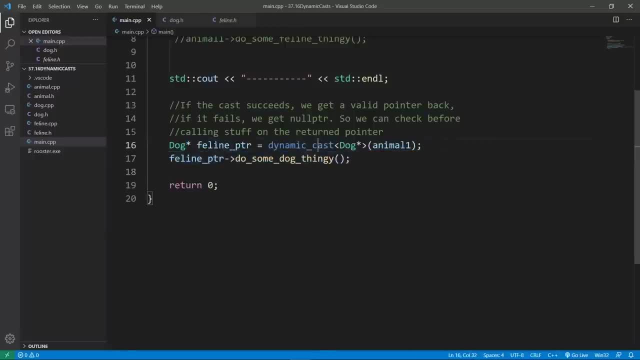 not going to give us any indication that we are doing something wrong. but if the transformation here fails, this is going to silently fail and store junk data in our feline pointer here, and here we're going to try and call a method that is going to possibly use. 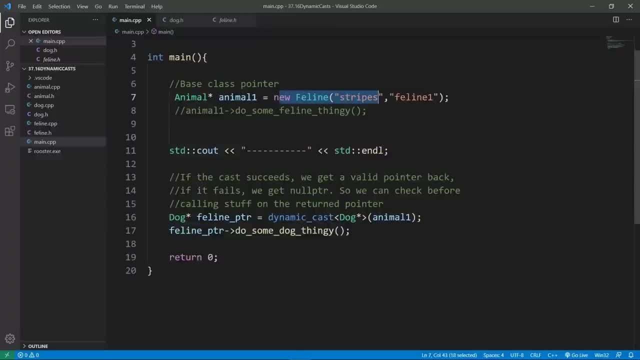 some dog stuff on the feline object. this is going to blow up again. we don't have dog information in this feline object and the do some dog thingy method is going to try and print the speed of the dog. that we don't really have. we don't have any dog information so we have no business accessing. 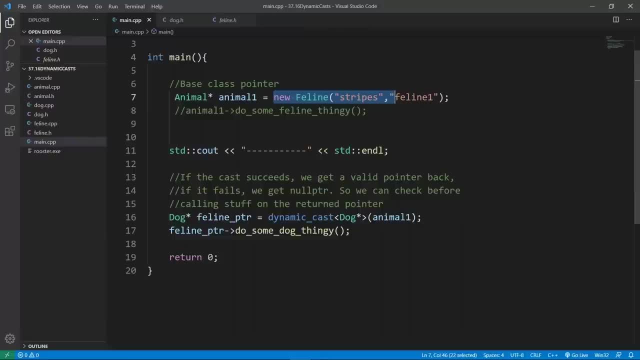 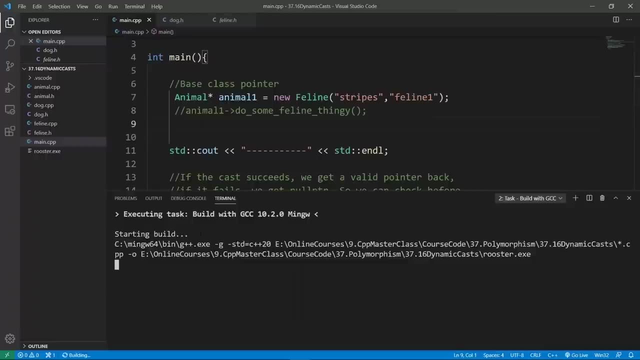 dog information from this object to start with. so this is going to blow up and it's probably going to give us a crash. let's try and build and see what happens. we're going to pass this through gcc, like we always do. the boat is going to go through. you see that this is going to even blow up at. 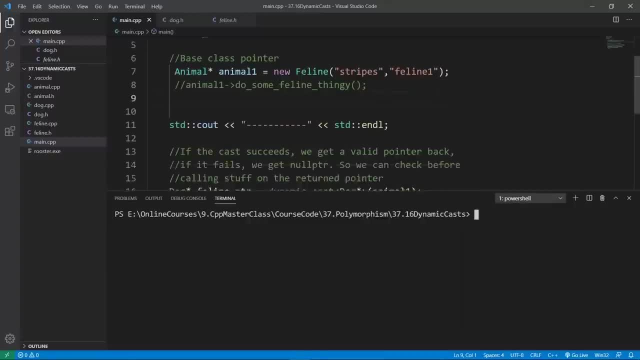 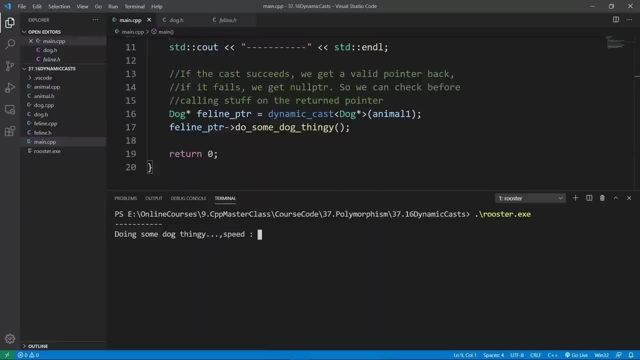 runtime when users are actually using your application. this is super dangerous. we're going to run this and see what happens. you see doing some dog thingy and it's going to try and print the speed. the compiler is really trying its best, but this is really going to fail and we are 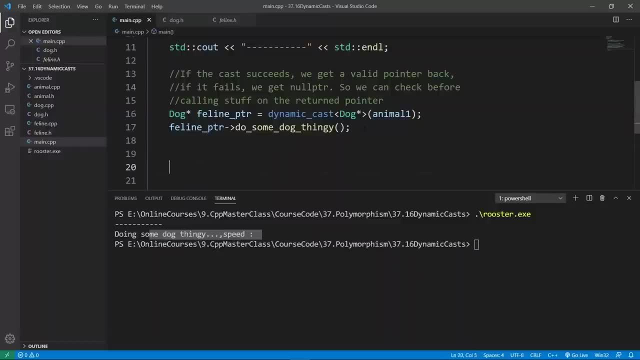 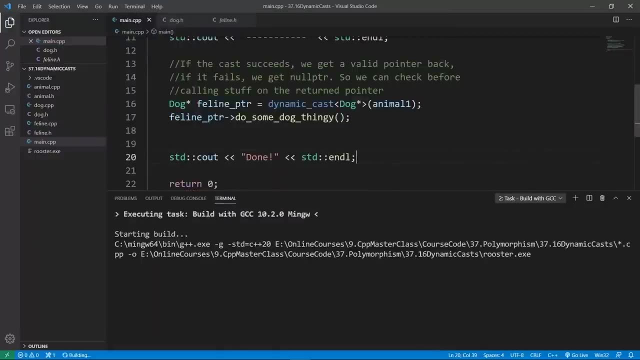 crashing our program if you go down here and say done, to make sure we know when the program is done and we try and run our program again. let's pass this through gcc to take into account this thing we have on line 20. the work is going to be. 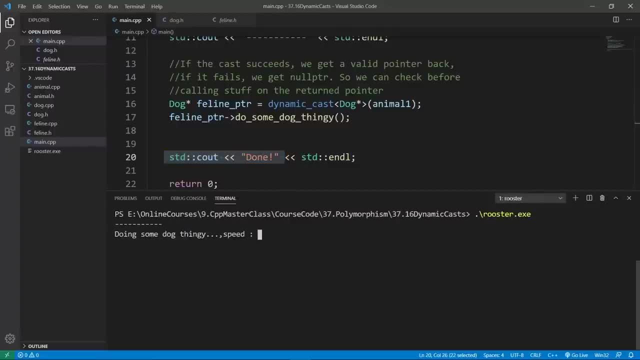 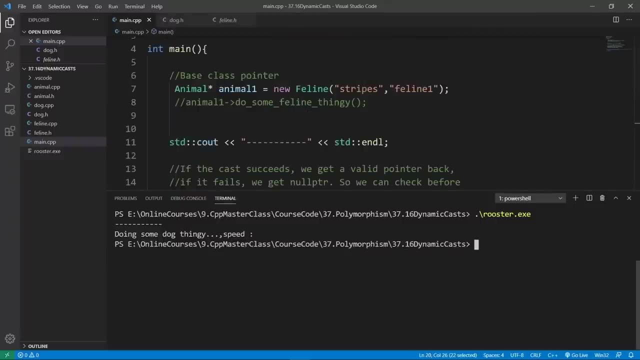 good, you're going to see that the computer is going to try and really run this, but it's going to see that it doesn't really have any dog information and the computer is not going to succeed because we are trying to access this dog specific information, really on a feline object. so 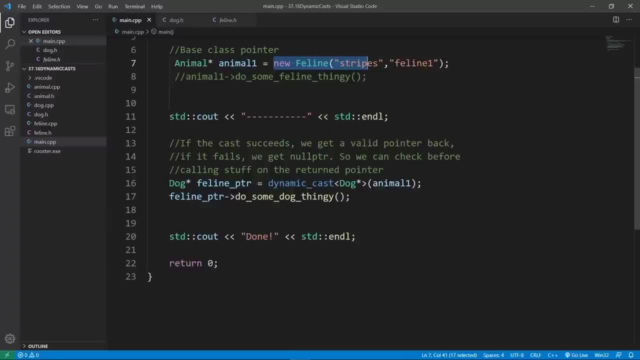 we are going to get a crash again. the message is that this dynamic casts can fail and we need a better way to do some kind of checks before we call our methods here, and we can do this by just using the pointer we get from this transformation here. so we 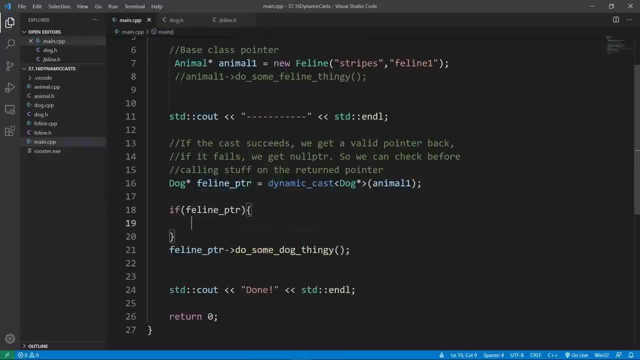 can say if feline pointer and check and see if we have some valid data in this feline pointer and if that's the case, we're going to do whatever we want to do with this pointer here. okay, so this is something we can do and if the transformation fails, 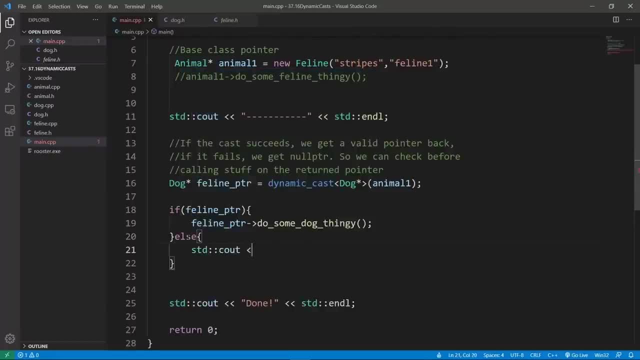 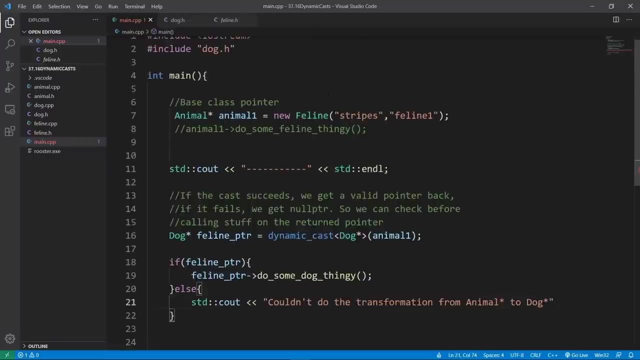 we're going to fall in this, else block and we can put some nice message here instead of letting the user crash at runtime. this is much better in my opinion. so we're going to say: couldn't do the transformation from animal pointer to dog pointer, because we really have no dog information in this. 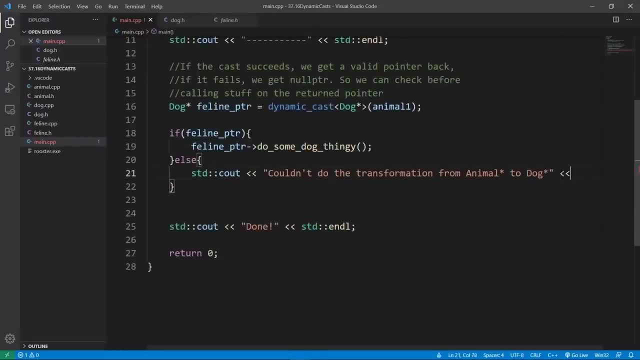 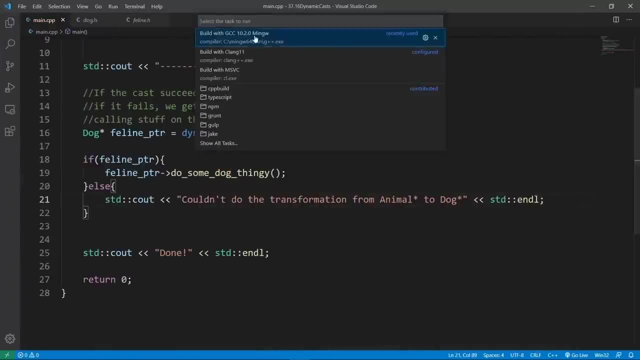 base pointer that we have here. this is something we can do, so we're going to say stdc out. we're going to say stdendl here and we're going to see what happens. let's bolt. hopefully we're ready to get the crash because we are doing something smarter. now we are checking to see if 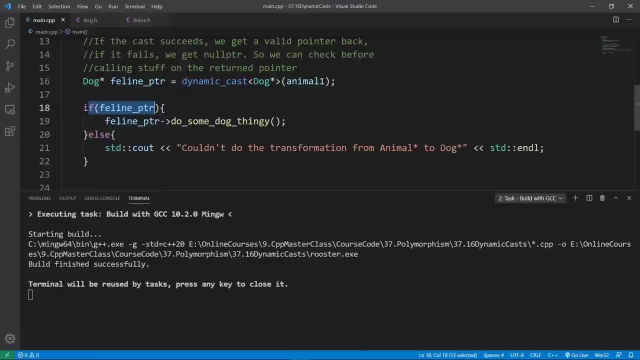 we have any dog information in this pointer. before we call some doubt specific method on this pointer here. this is the beauty of this. we're going to clear and run rooster now. you see, couldn't do the transformation from animal to dog and our program is no longer crashing, it is ending. 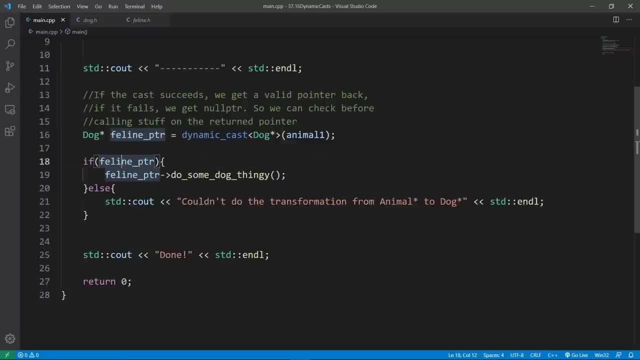 properly and this is much better. this is what you should aim for. so again, the transformations here. but if we turn this back to doing feline transformation, let's do feline pointer. we're going to change this to fill line pointer again and we're going to do some feline thingy. now we're 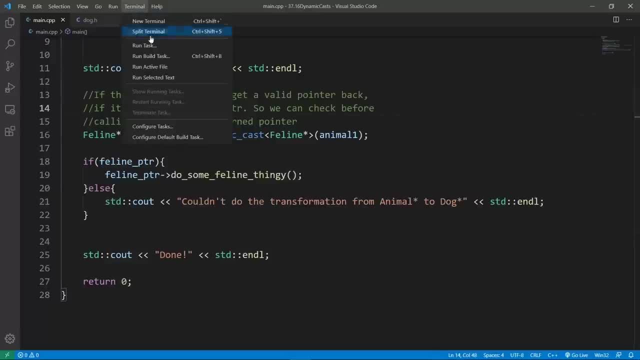 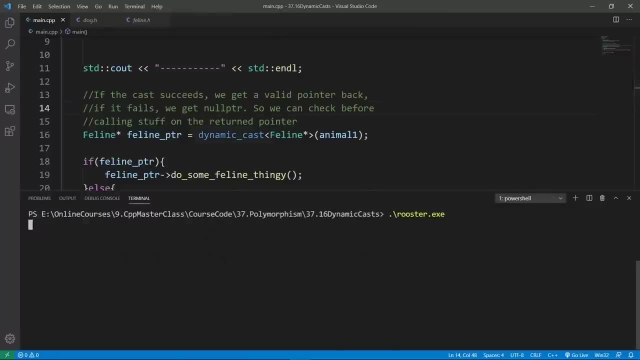 going to build again, and this is true. we're going to build again and this is going to build successfully and it is going to properly do some feline thingy. the build is good, we can clear and run rooster. this is going to work just fine and our program is going to end properly. so here we. 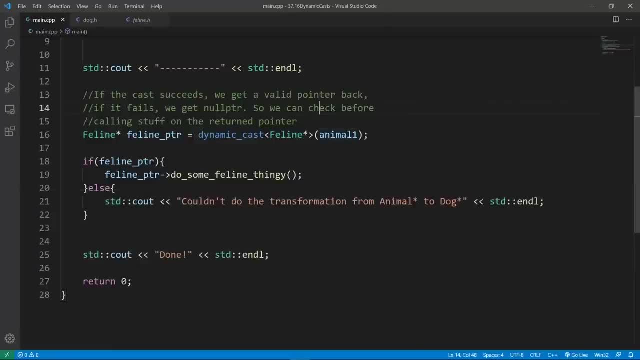 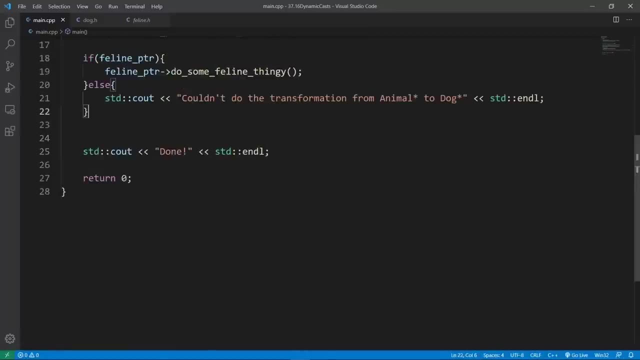 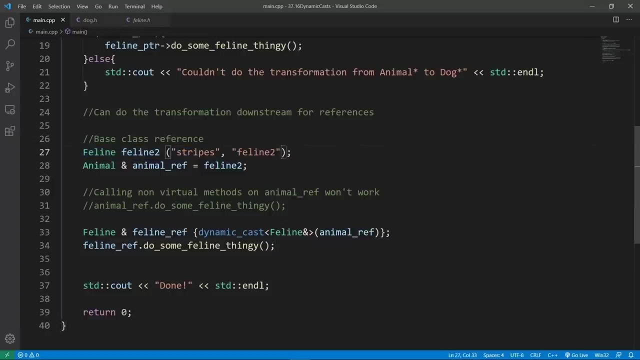 just saw that we could do a transformation from a base pointer to a derived pointer and this is going to work just fine. we can also do the transformation for references. let's say that here and we're going to go down and put in a simple example to drive this home: we're going to have a feline object. we're going. 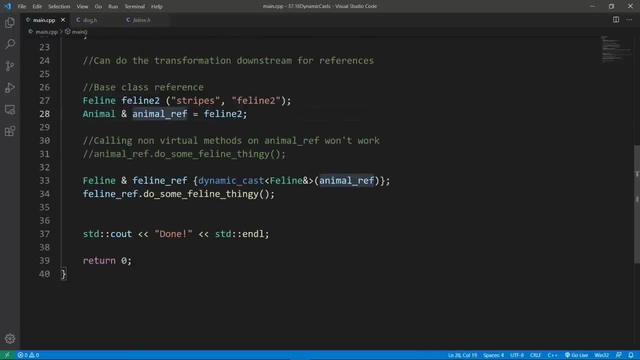 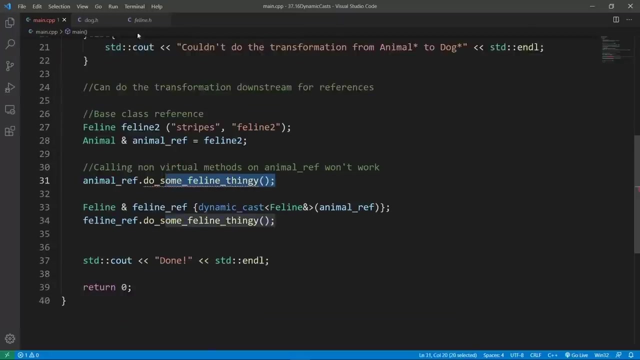 to set up a reference to it and if we try and call a non-virtual method on this base reference, this is going to blow up because the base class has no information about this non-virtual method. that we we're at the feline level. this is going to blow up. if we're trying to build our program, we're going. 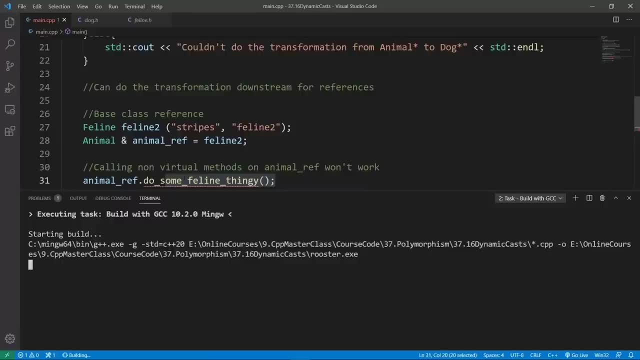 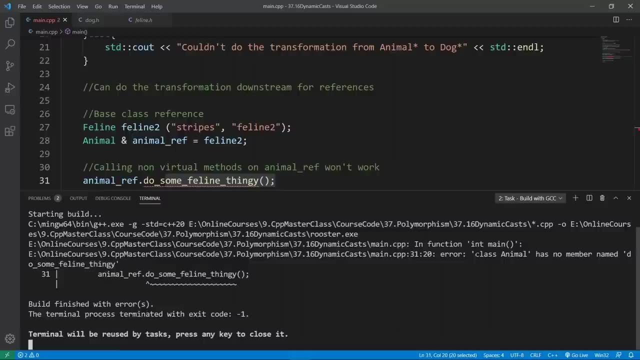 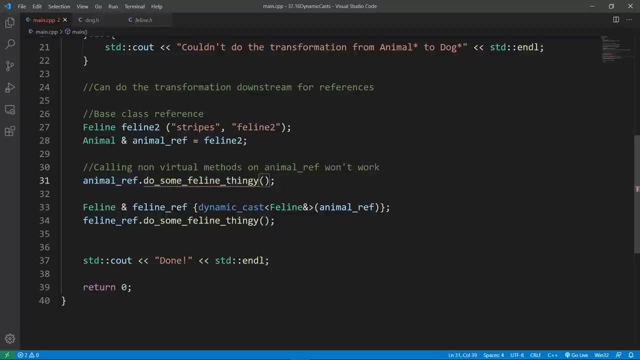 to see that we get a compiler error saying no such method as do some feeling thing. we're going to see that here no member named this way at the animal level. this is the compiler error we get if we try to call a non-virtual method through a base reference that we have here. this is not going to. 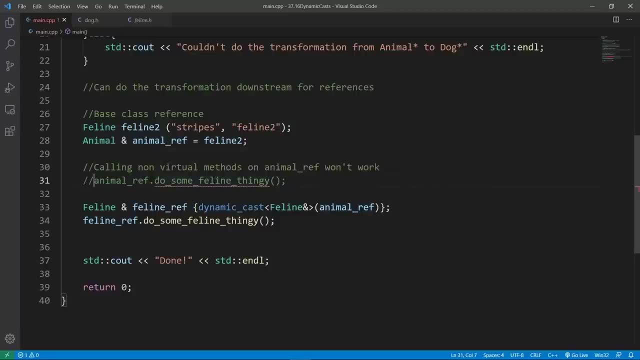 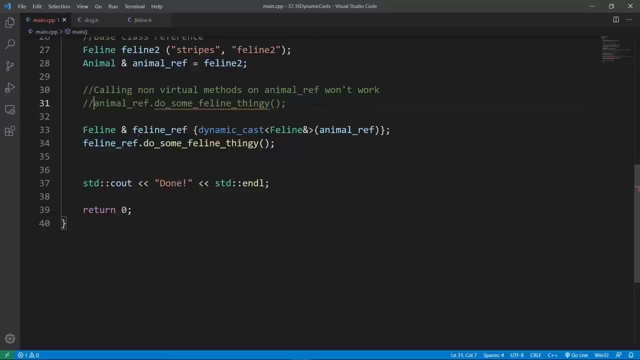 work. but we can also do a dynamic cast and transform from a base reference to a derived reference, and the syntax to do that is really here. we're going to set up a derived reference- in this case it's going to be a feline reference. we going to initialize this with a dynamic cast transformation and the result of the cast is: 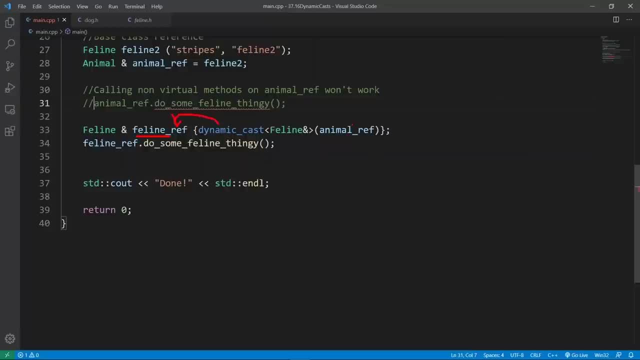 going to be used to initialize this reference here and we're going to be taken a base reference and turning that into a derived reference here. this is the syntax: the outputs you desire is going to be within this angle brackets and the input is going to be through this parenthesis here. if 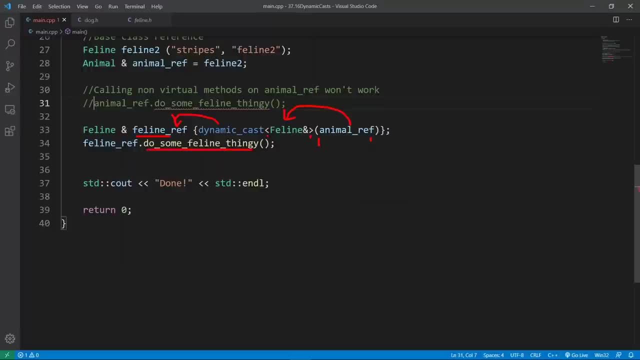 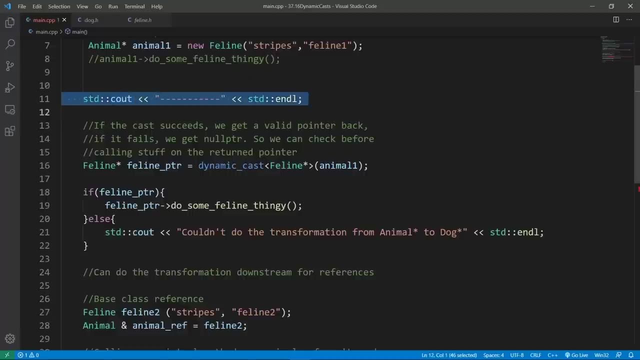 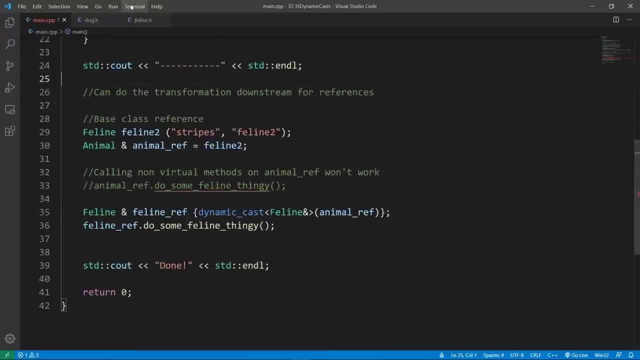 this succeeds, we will be able to call our method here and this is going to work just fine. let's try this out. we are going to put in a separator to be able to follow these things. let's put that at line 24 here. this is going to do and we're going to try and build our program. we're going. 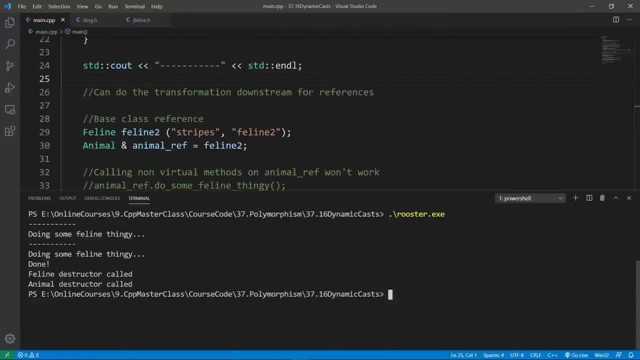 to pass this through gcc. the both is good. we can clear and run rooster. now we're going to see that we are doing some feline thingy through a reference and this is super cool. we can do this, you can do this kind of transformation here, and at the end you see that we are calling our 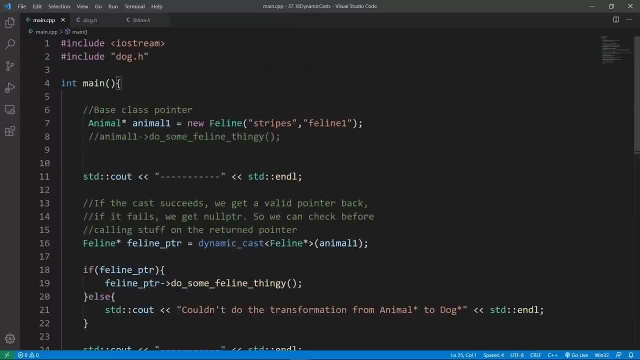 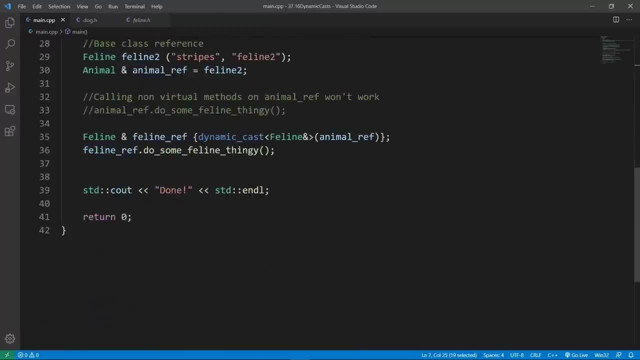 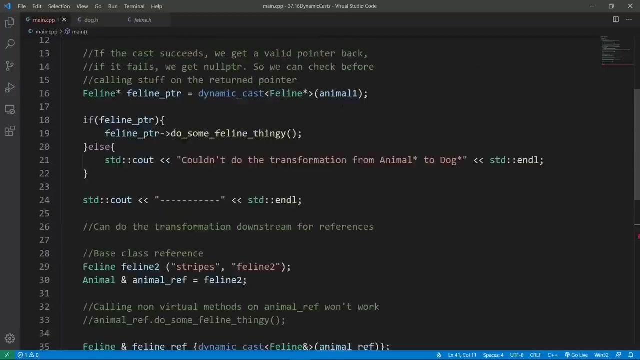 destructors on our objects and this is a good reminder that we didn't properly release the memory on this animal pointer that we had. so we are going to go down at the end of the program and release that memory. this is good practice and hopefully you can see how easy it is. 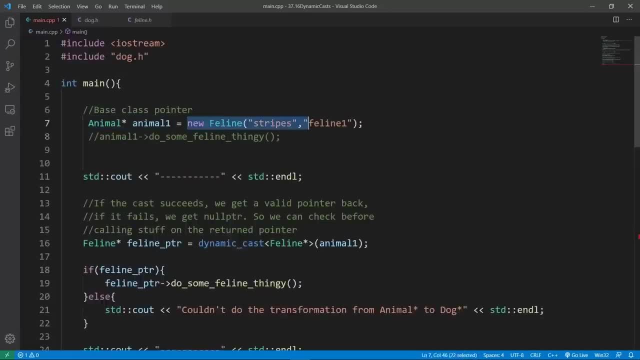 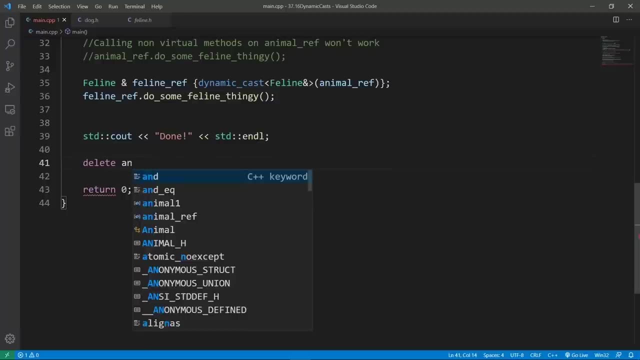 to forget to release some memory that you allocate for with the new operator. this is a good learning experience here. but this is a good learning experience here. but we're going to fix this problem. we're going to say animal one and we're going to release the memory. now, if we run the 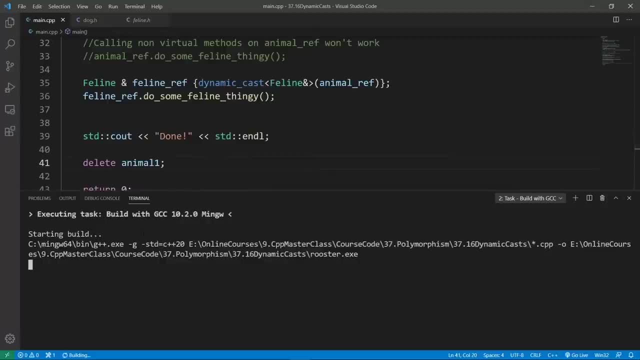 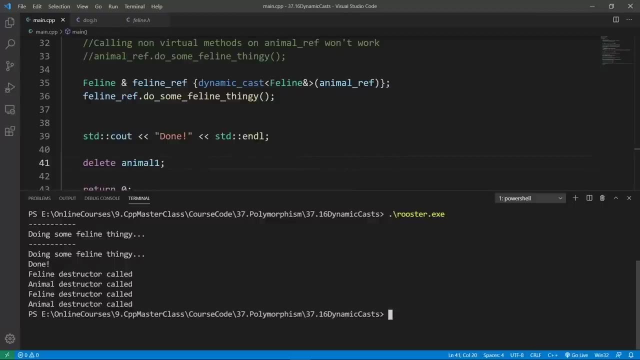 program, we're going to see that we are releasing two objects. when the program ends, we're going to clear and run rooster and the destructor is going to be called two times: once for this guy and a we want. and you see that because we have virtual destructors in our classes, we are destroying at. 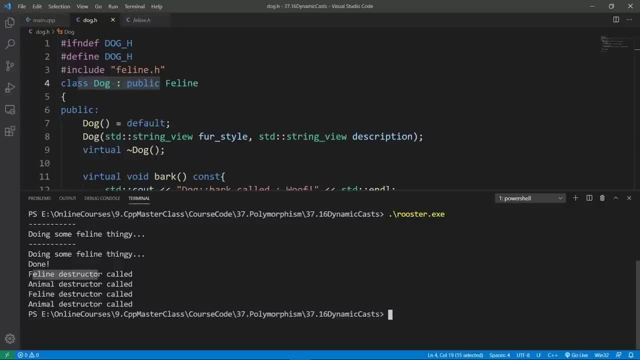 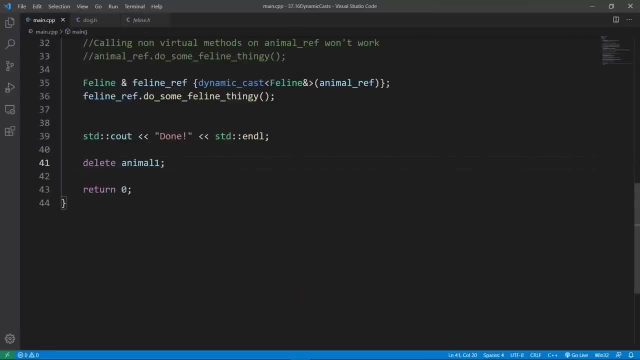 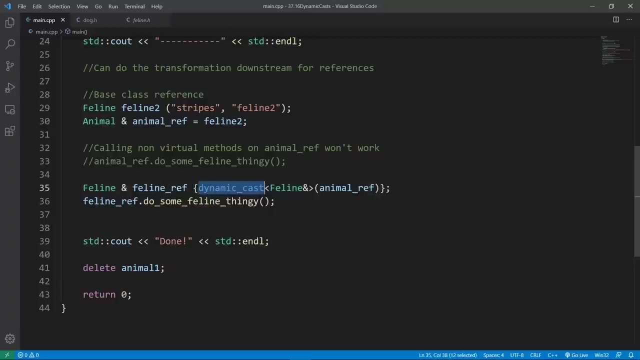 each level. so here we are destroying at the feline level and we are destroying at the animal level, and this is going to properly release the memory from our inheritance hierarchy here. so now you know that you can do a transformation of references using dynamic casts, but with dynamic cast we have 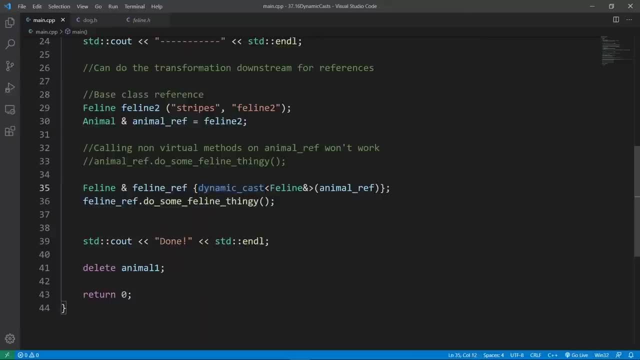 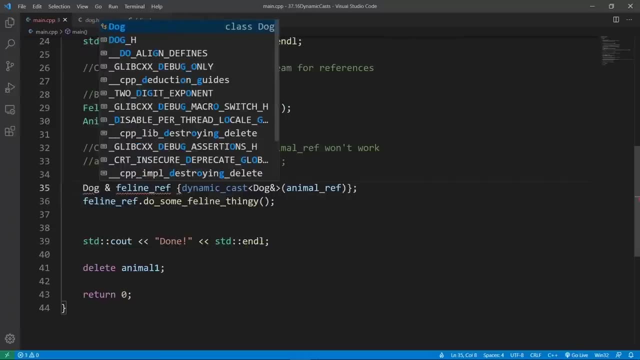 no way to check and see if the transformation was successful. again, if we try to turn this into a dog reference, we can do that and we're going to say dog reference here and we will try and call the do some dog thingy method. this is not going to give us an 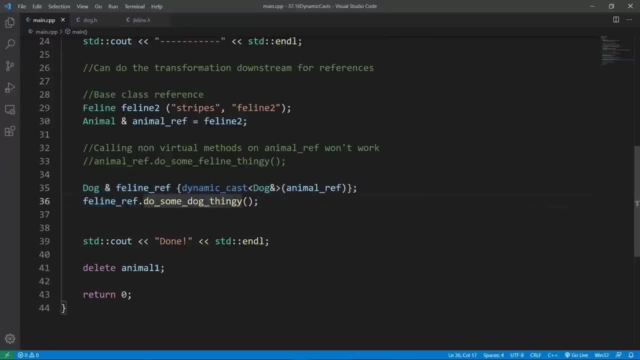 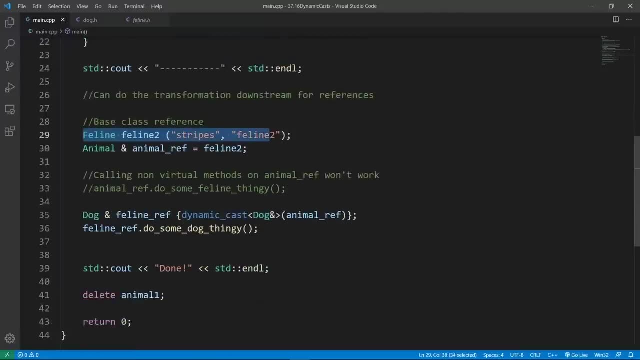 indication of a problem, but this is going to crash at runtime because we don't really have any dog information in our original feline object here. so if you try and transform this reference into a dog reference, this is obviously not going to work because we have no dog information in this. 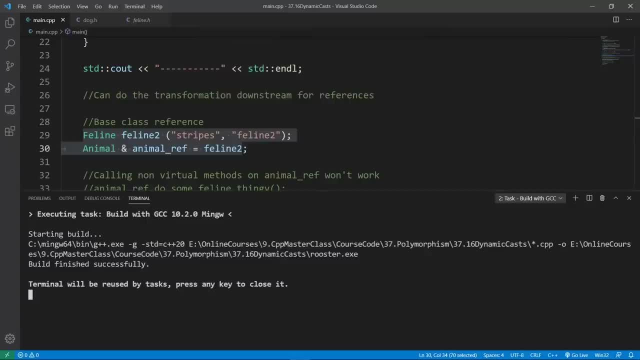 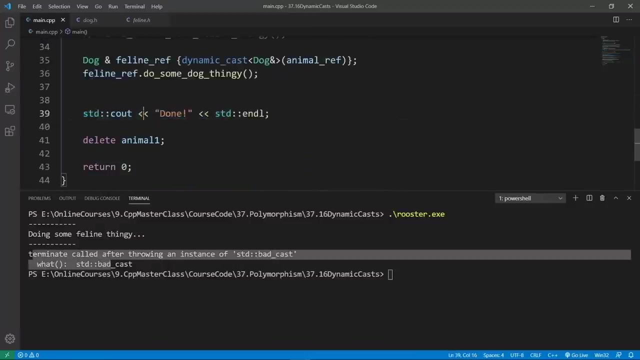 to start with, let's build and show you the problem. the book is going to be good so we can clear and run rooster. you're going to see that we are going to terminate our program with a bad cast and this is going to crush. you see that we don't get to the point where we print done and we are not even going. 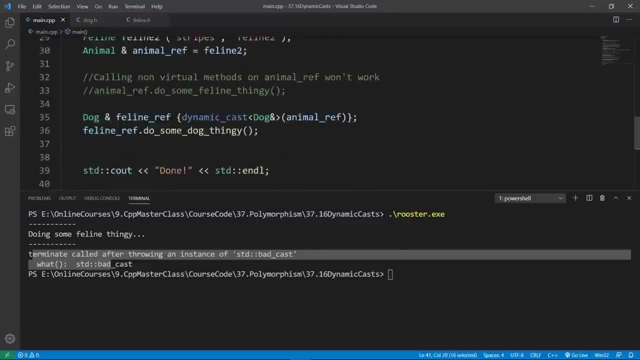 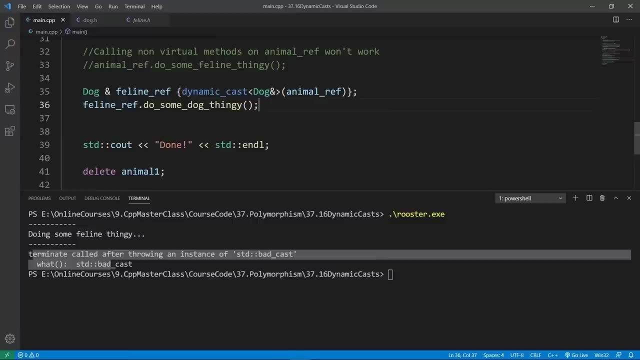 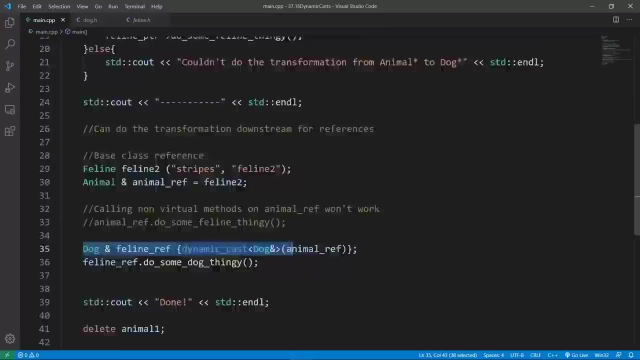 to get a chance to release the memory that we have allocated in this main function. hopefully you can see that this is really bad. so with references, we have no way to check and see if the transformation was successful, and this is a limitation. that's why, in most cases, I usually do. 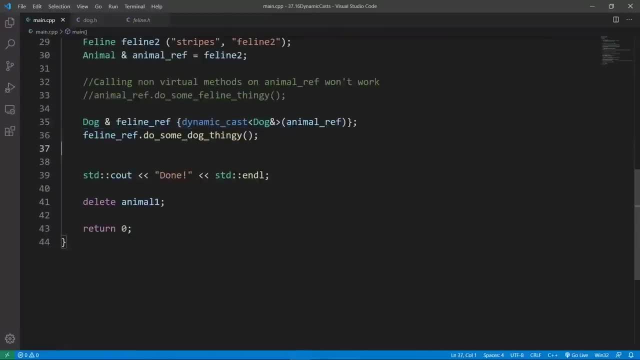 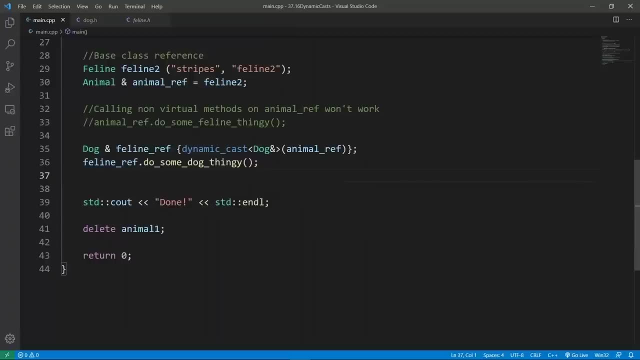 my transformations through pointers and there is a way you can even turn this base reference into a base pointer and I am going to show you how you can do that. so we are going to go down here and try to change things a little bit. we are going to say: doing proper checks with references and 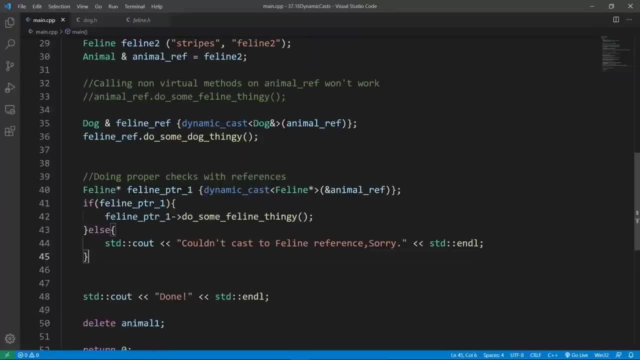 we're going to put in a piece of code to play with us and what we're going to do. we're going to take the reference and turn that into a base pointer. this is the syntax. here again, the input is a base reference, but the output we desire is a base pointer, and this is possible in c++. this is going. 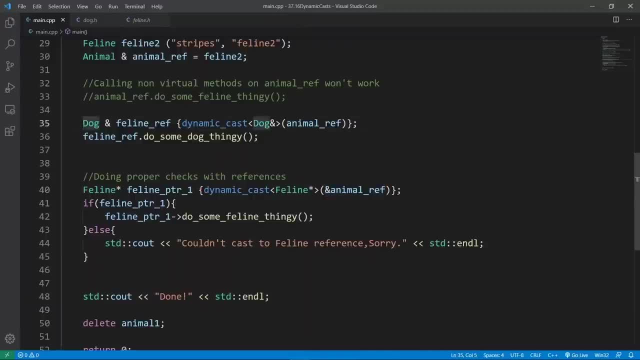 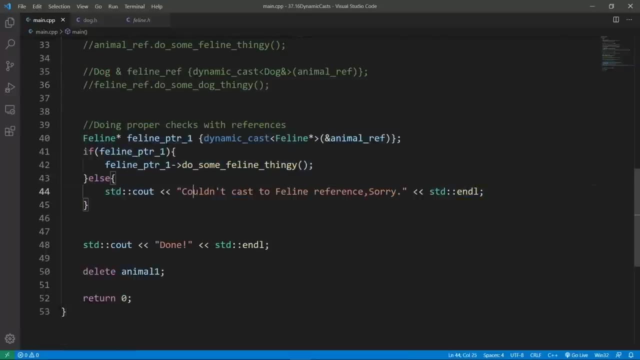 to work just fine. now we are going to go on top and comment this problematic transformation we just tried to do and we're going to try and build and see if this is actually working. if this transformation succeeds, we're going to do some feline thingy. if it fails, we're going to say: 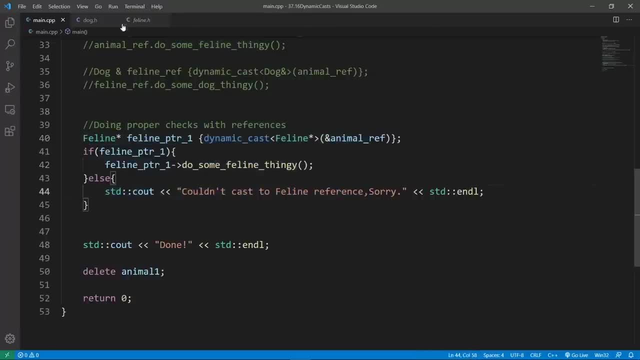 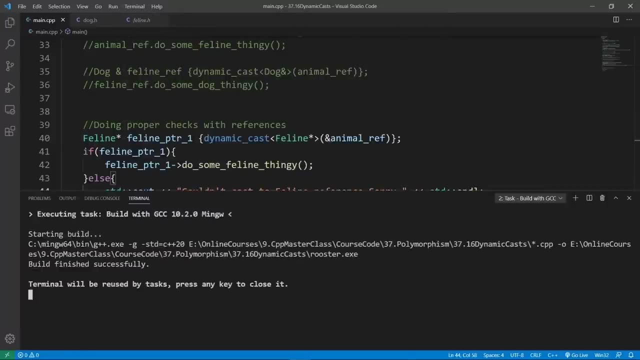 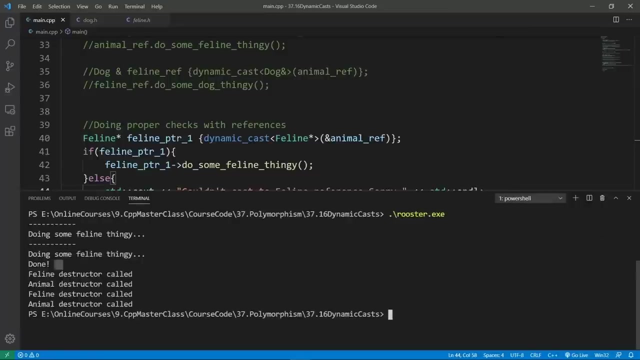 couldn't cast to feline reference and we're going to say that we are sorry. this is a good output message if we get something wrong. we're going to build this with gcc and see if this actually works. the build is good. we can clear and run rooster. you see that this is working just fine. we're going to 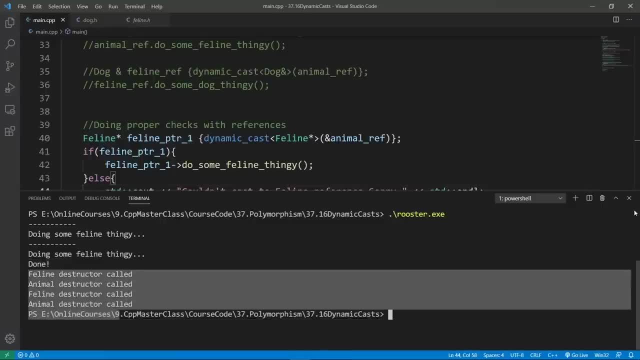 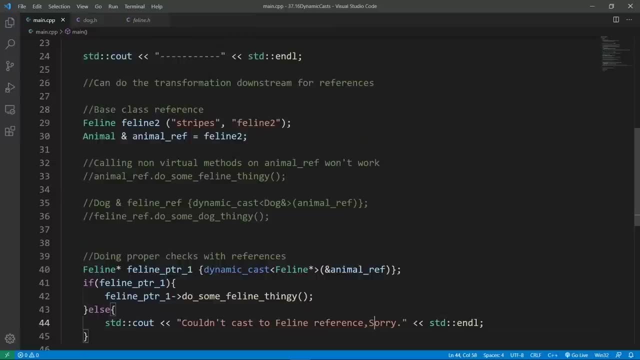 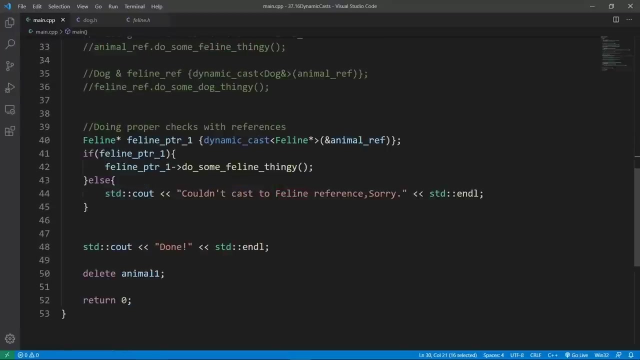 hit the end of the program and we are going to destroy our objects here. this is super cool, but if we try and do the transformation and transform to a dog object, even if we know that we don't have any dog information in this object that we are referencing to start with, we hope that we're 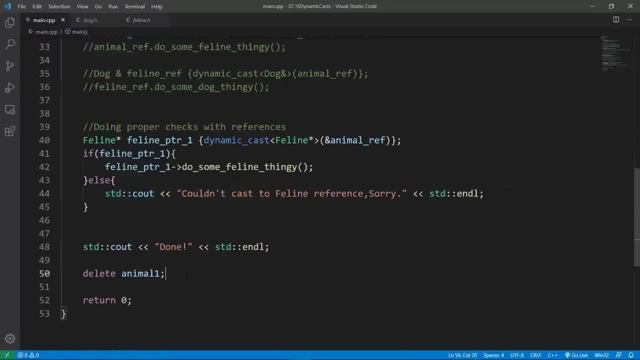 going to get a good message and the program is going to end properly. we're not going to get a crash, so let's make sure we are transforming to dog here. we're going to pass a dog pointer as our output and we're going to store this as a dog pointer, even if the name is still feline pointer. 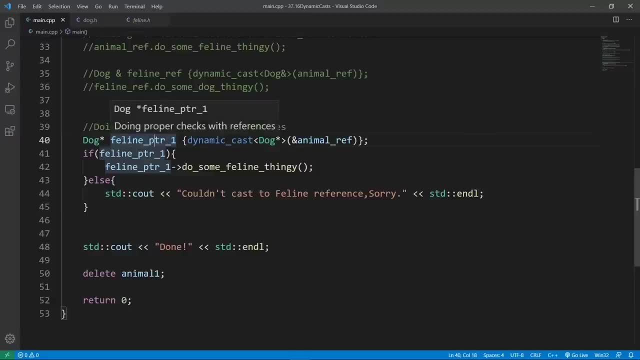 hopefully this is not going to confuse you. even if this is named feline pointer, it is a dog pointer here because we just want to see if we get the error message that we have here. so we are turning this reference into a pointer and the benefit of this is that a pointer can store no pointers and we can use 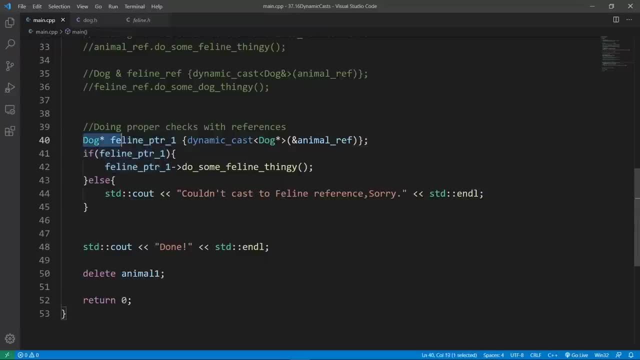 this to our advantage to check and see if the transformation here was successful. if it was successful, we will call some dog then method. let's say that here, and if this fails, we're going to say that we couldn't transform to dog, and this is going to give us a nice message and 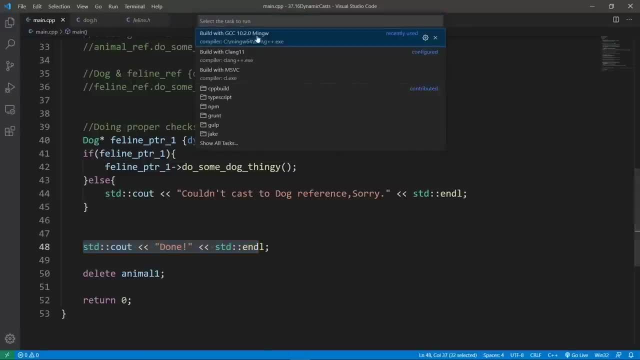 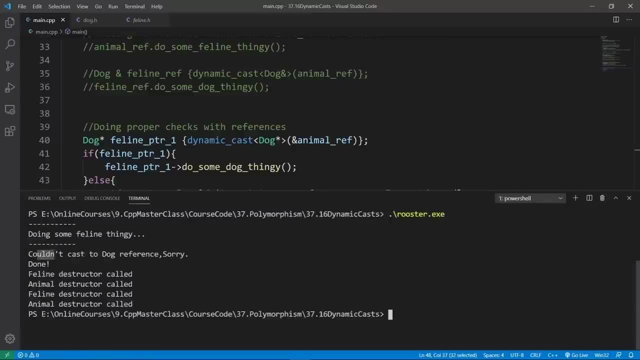 our program is not going to crash. we're going to build this again with gcc. well, it's going to be good. as you see, here we're going to clear and run rooster. now you see that we are saying we couldn't cast the dog reference and our program is not crashing. so if you have a reference to start with, 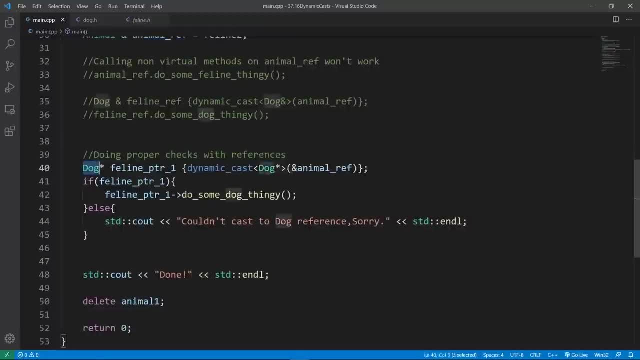 and you want to do some proper checks after you do the transformation to a derived pointer or a derived reference. this is the best of both worlds. you can do something like this and your program is going to be much safer. the last thing we're going to do is we're going to go to our program and we're 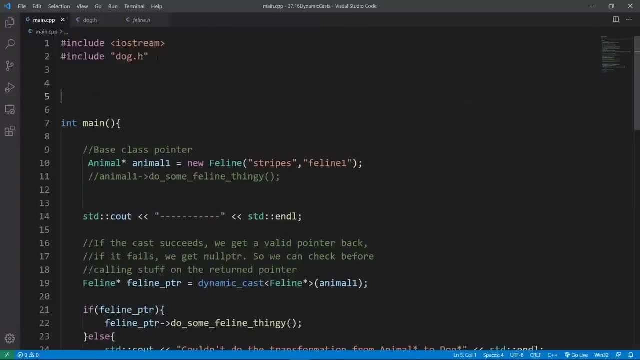 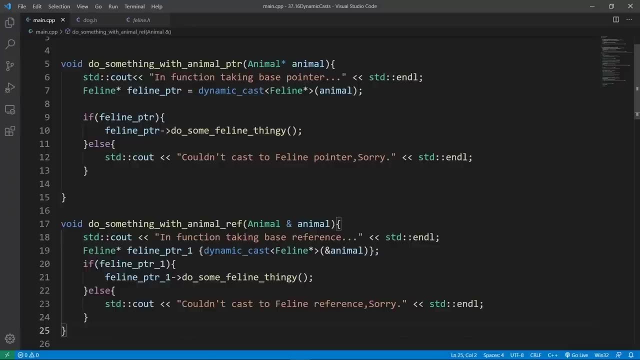 going to run the on. the first thing i want you to see is that these kinds of dynamic casts are really useful if you are passing base pointer or base references into functions. and here i am going to put in a bunch of functions. the first one is going to take a base pointer. the second one is: 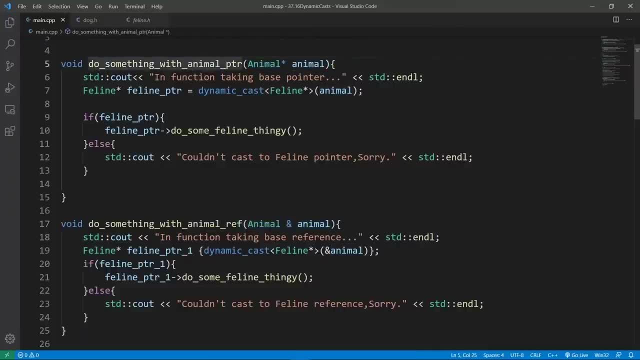 going to take a base reference and it is going to say: do something with animal pointer and do something with animal reference, and inside we're going to do our thing here. we're going to take the animal pointer, turn that into a feline pointer and we're going to do our proper check and we're 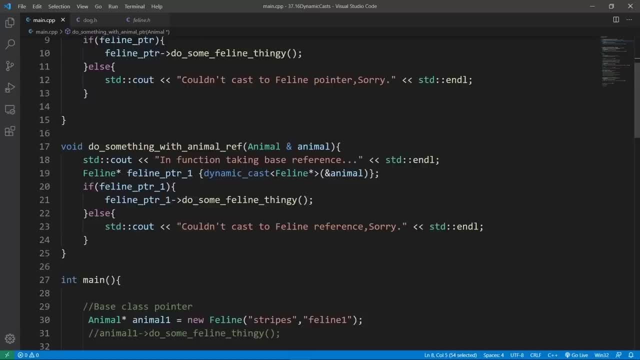 going to do some feline thingy if the transformation was successful. we can do something like this. we can also do exactly the same thing with references. we're going to take our input reference, we're going to turn that into a derived object and we can call our method on this pointer. 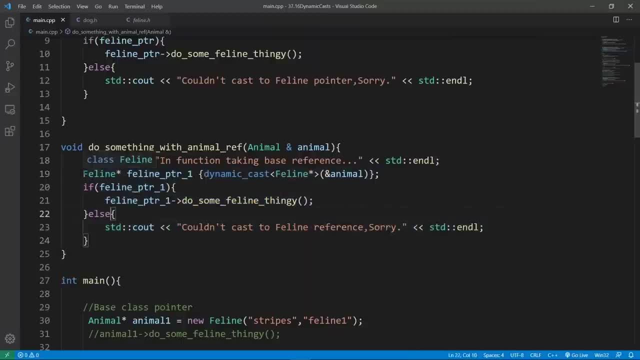 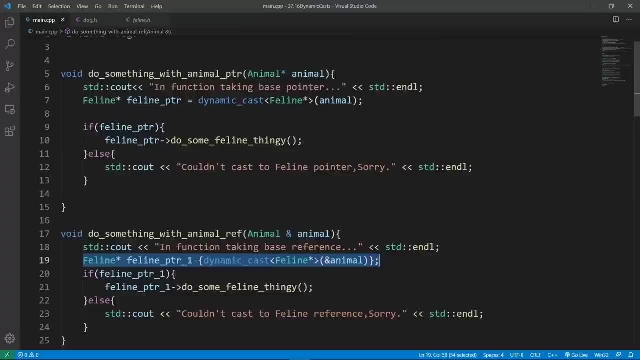 and we're going to do proper checks, because we have a pointer which has a concept of null pointer that we get if the transformation here fails. this is the setup we can use in our c++ programs and we can use these methods to get derived pointers that we can call even non-polymorphic functions on. 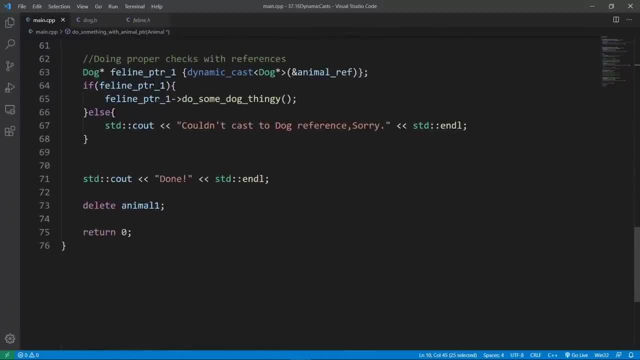 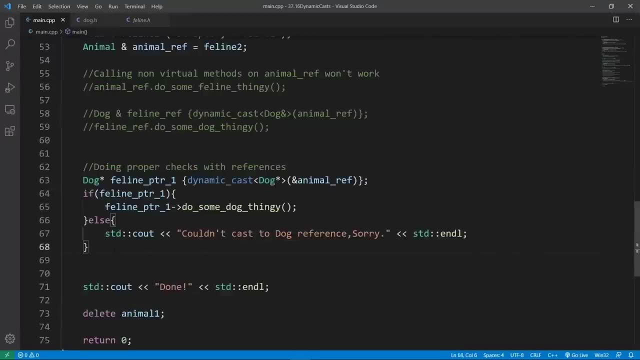 and this is going to work really well, so we can go down and comment out everything, i guess to make this super easy to follow. but i don't think we need to comment out everything. we can just comment out what we just did here and we're going to be reusing the reference we have here and the pointer. 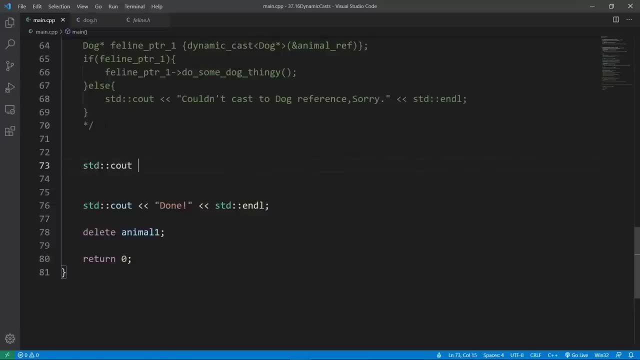 we have all the way to the top. so we're going to go down and put in a separator here. we can do that and because of this separator i don't think we even need to comment things out. we can remove our comment and leave the code in. 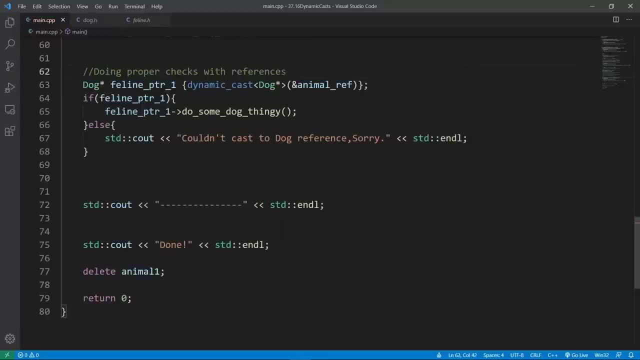 because i want you to see that super easily and we're going to call our functions here. we're going to say: do something with animal pointer. and we're going to pass an animal one which is a pointer, and we're going to say: do something with animal ref. okay, do something like this. and we're going 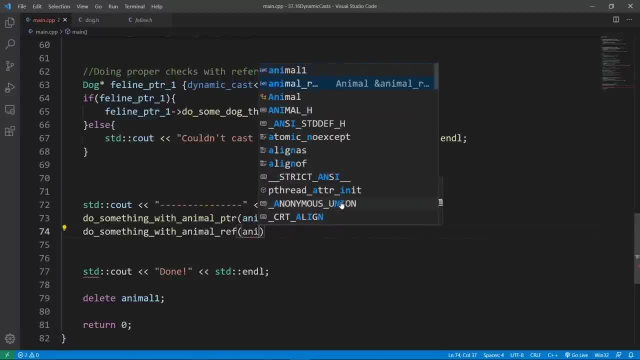 to pass an animal ref. we have this reference here and we can do something like this. you're going to see that this is not going to give us any kind of problem and it is going to work just fine. let's bold. we're going to pass this through gcc. the bold is going to be good. we can clear and run rooster. 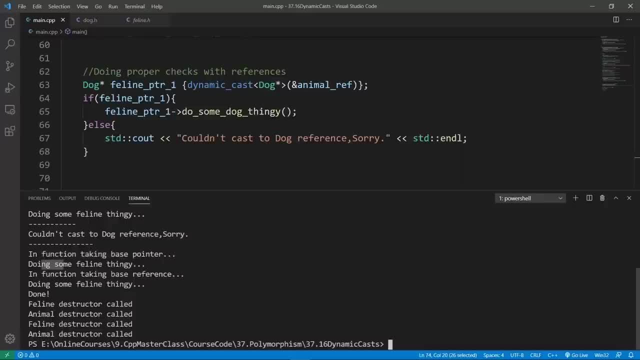 and down here you see that in function, taking base pointer doing some feline thingy, in function, taking some base reference doing some feline thingy, and this is working really fine. this is what we want in our c++ programs. this is really all i wanted you to see in this lecture, hopefully. 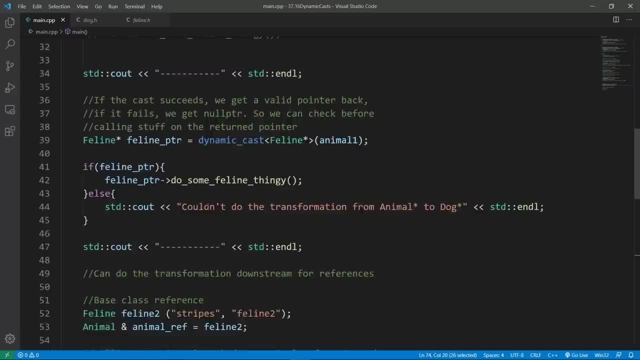 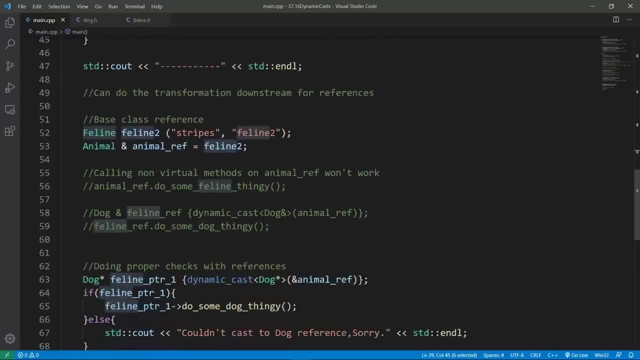 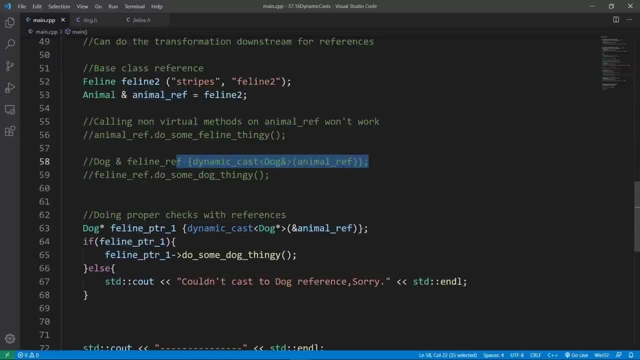 you didn't find it confusing. again, the message is that you can do dynamic casts to transform from a base pointer to a derived pointer or to transform from a base reference to a derived reference, as we did right here. but transforming to a derived reference has a drawback in that you don't have a way to check and see if the transformation was. 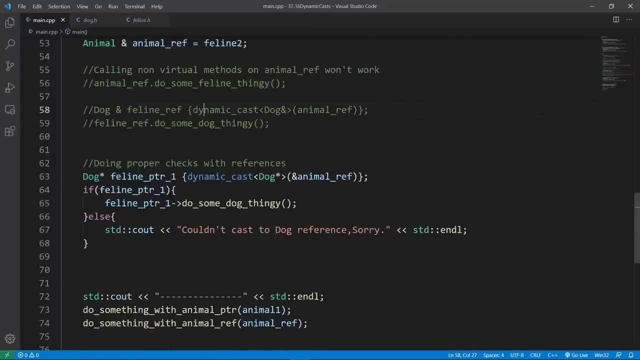 successful. so if you want to be able to do checks, you can do something like this and turn a base reference into a derived pointer and then we can check and see if the pointer is not a null pointer. if it's a null pointer, we will note that the transformation failed and we will print a good error message if the transformation was. 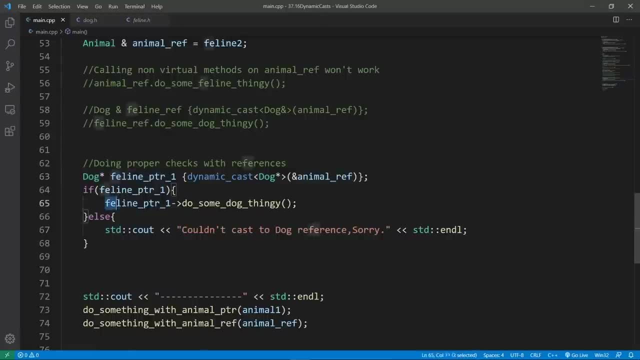 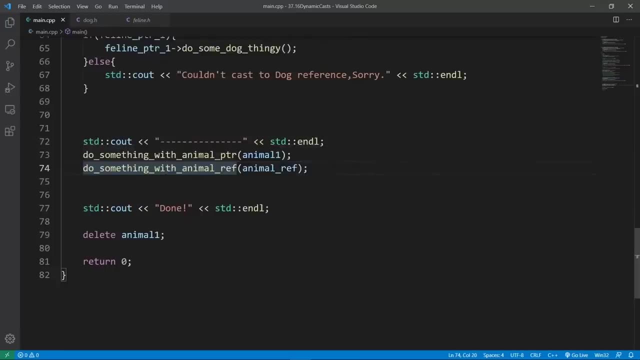 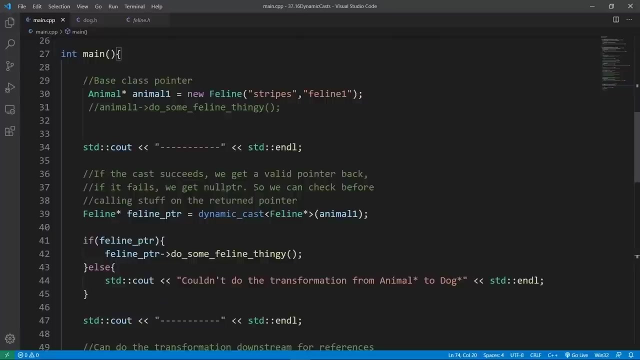 successful, we will have a valid pointer in here and we will call our derived non-polymorphic method on our pointer. this is going to work really fine. the last thing i want you to see before we wrap up this lecture is that dynamic casts are only going to work with polymorphic inheritance hierarchies. 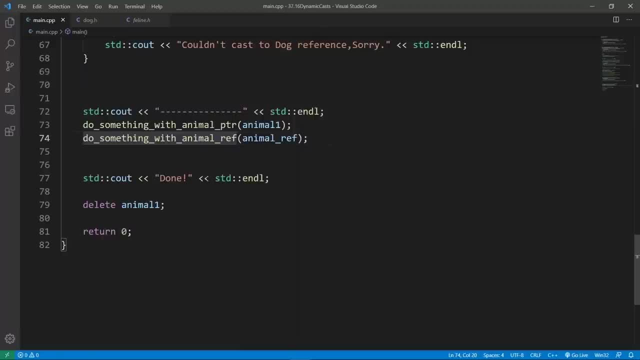 so, for example, if we try and turn a double into a strength, obviously that's not going to work with a dynamic cast. but let's try and do that to really show you that this is going to give us a problem. we're going to say std cout, and we're going to put in a separator here and we're going to set up. 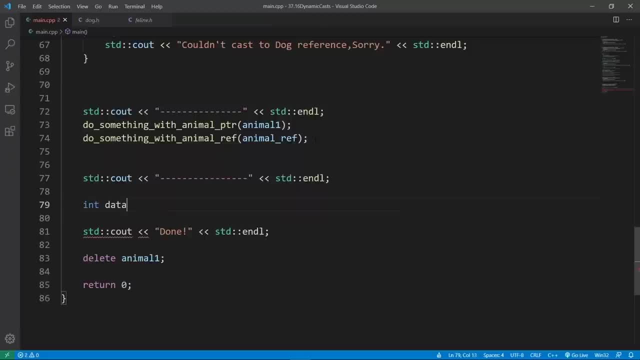 two variables. one is going to be a net, for example, and we're going to say data, we're going to put in a 45 and if we do a dynamic cast to an std strength, for example, that's not going to work. we're going to say std strength, yeah, and we're going to put in a separator here and we're going to put in a. 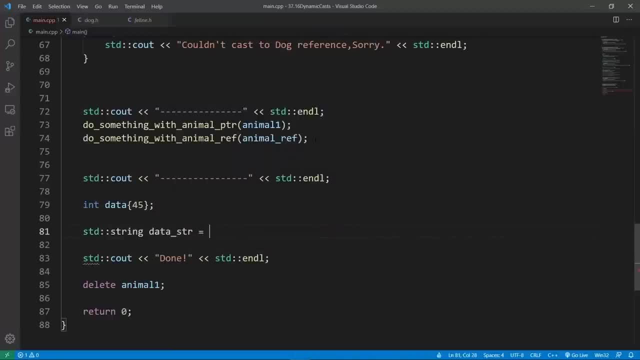 str, meaning that this is a string. we're going to say dynamic cast. let's say we want to turn this into an std string, for example, and the input is going to be our data. if you're trying to do something like this, this is going to blow up. you see that even visual studio code is giving us a. 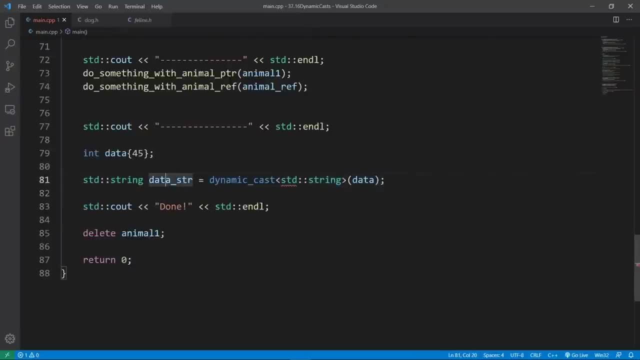 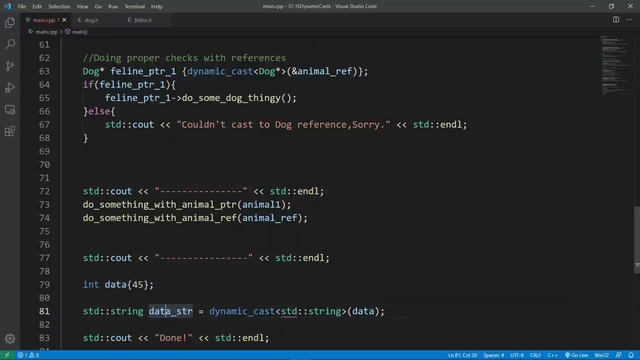 squiggly line, so this is not going to work. just make sure you use dynamic casts in an inheritance hierarchy that supports virtual functions. this is the design purpose for the dynamic cast. if you use this outside this context, you're going to get undefined behavior or even compiler. 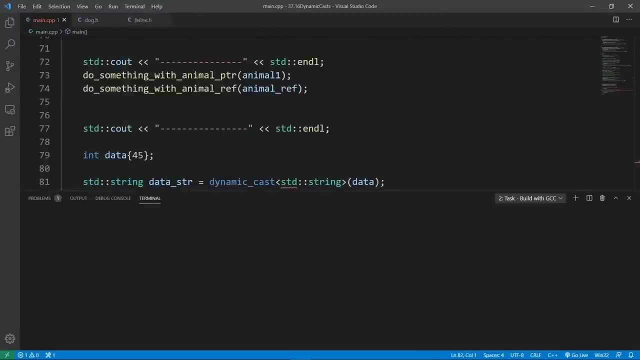 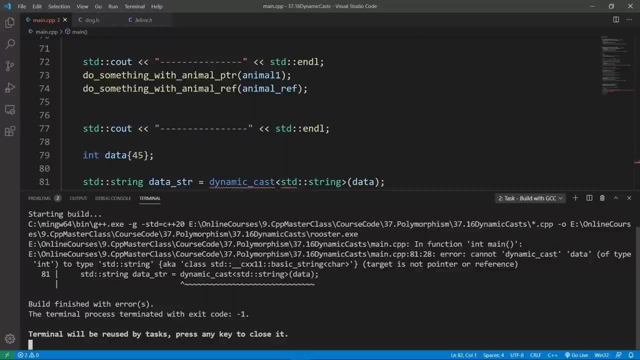 errors. if you are lucky, let's try and weld and show you this. we're going to pass this through gcc and we're probably going to get an error saying that we can't transform from an integer to a strength, for example. let's go here: cannot dynamic cast. so basically it is saying dynamic casts are. 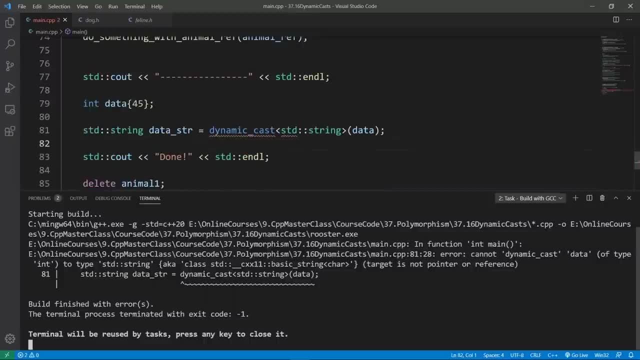 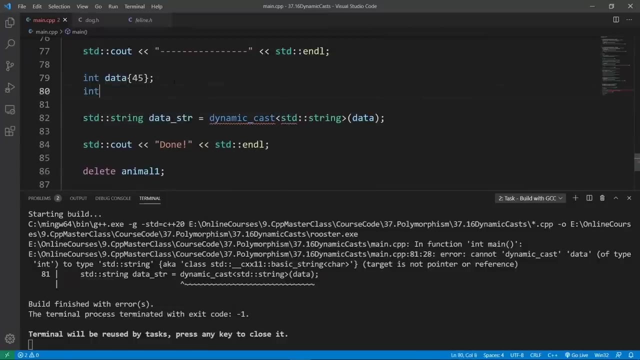 meant to work only with pointers or references, but even then let's see if we can transform from an end pointer to a string pointer. let's try and do that. let's say we want to turn the address of data, or let's set up a pointer. to be explicit, we're going to say 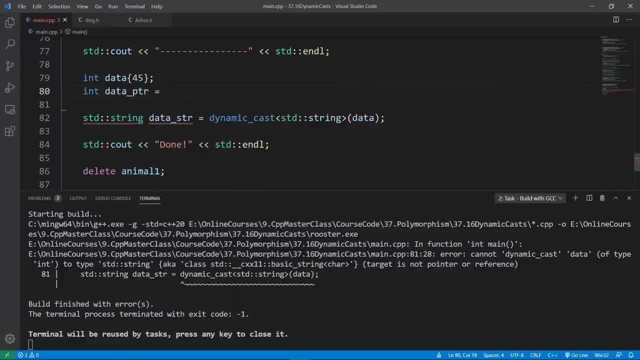 data ptr and we're going to initialize this with the address of data. we can do something like this and we're going to cast data ptr to an std string pointer. let's see if we can do this, because it is meant to cast between pointers and references. but you see that this 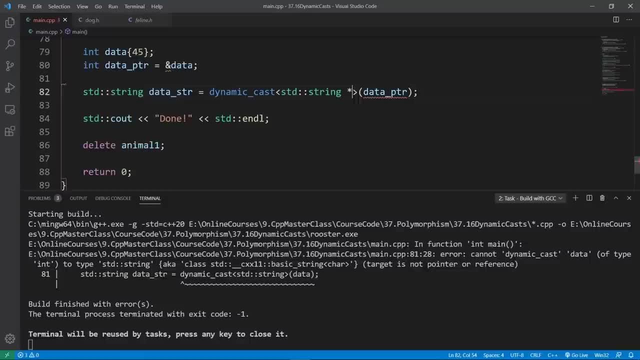 is even not going to work. so you shouldn't really do something like this if your input and output are not part of the same polymorphic inheritance hierarchy. again, dynamic casts are meant to cast from base information to derived information, and the input and output must be part of the same. 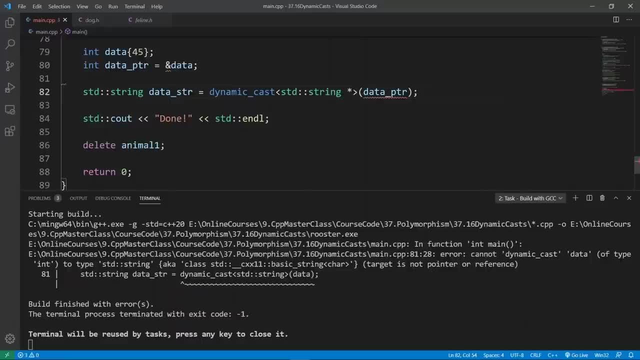 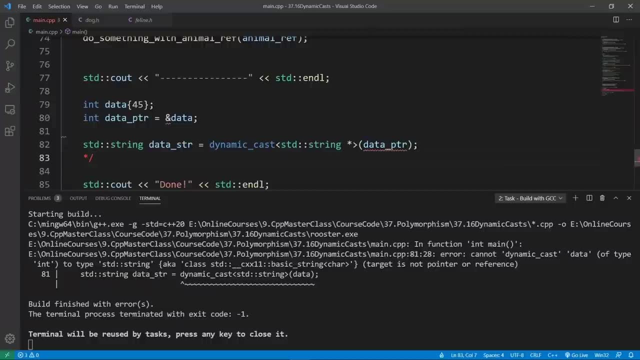 polymorphic inheritance hierarchy. this is the information i am trying to convey here. so this is bad. don't do something like this. if you do this, you're going to get undefined behavior or you're even going to get a bunch of compiler errors. if you are lucky, this is really all we set out to do in this lecture: showing you that you can use. 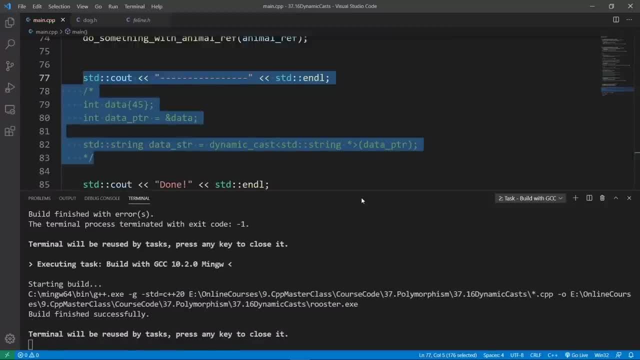 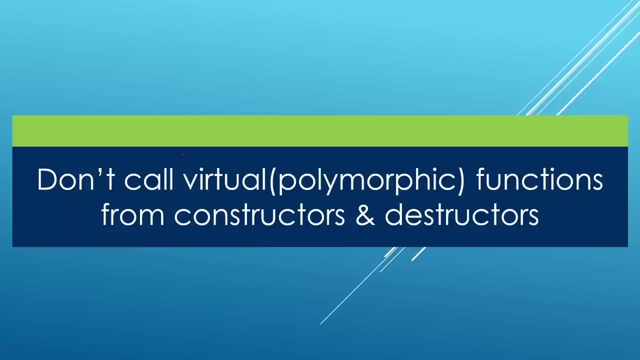 dynamic casts. we are going to stop here in this lecture. in the next one we're going to show you what happens if you try to call a polymorphic function from a destructor. go ahead and finish up here and meet me there. in this lecture i am going to give you a warning, and that is to never call. 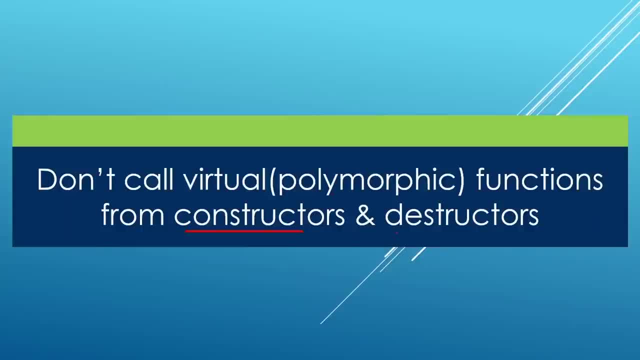 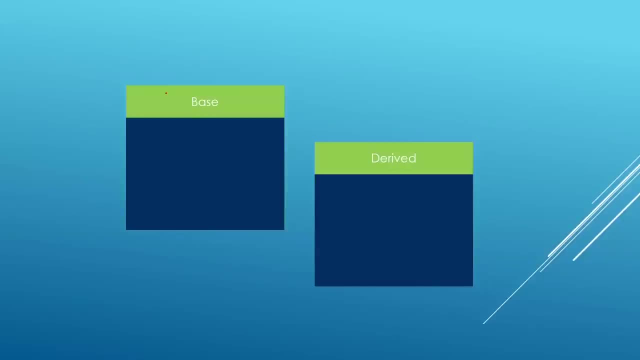 virtual functions from constructors or destructors. i am going to repeat this never: never call virtual or polymorphic functions either from constructors or destructors, and we're going to explore why we're going to be using this inheritance hierarchy. we're going to have a base class called 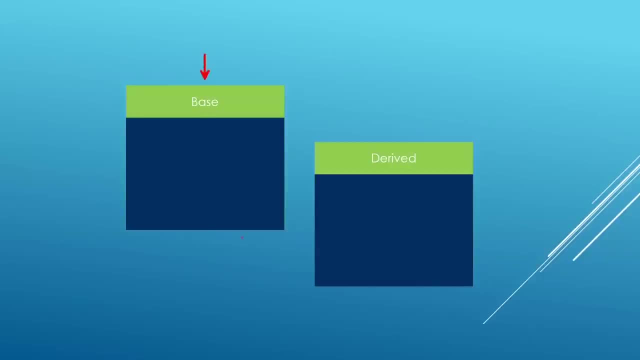 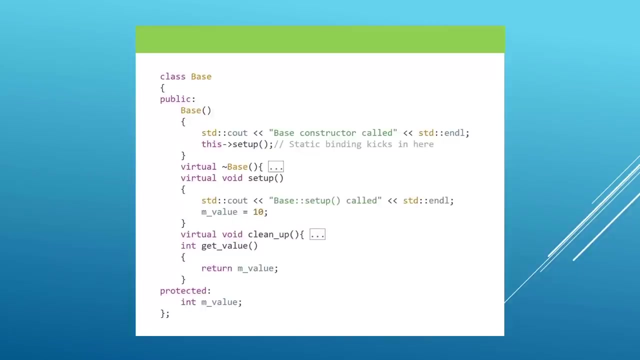 base, how creative. we're going to inherit from base and create derived, which is our inherited class, and we're going to be using this to explore why we can't call virtual functions from constructors and the instructors. this is what our code is going to look like. the base class is going to have. 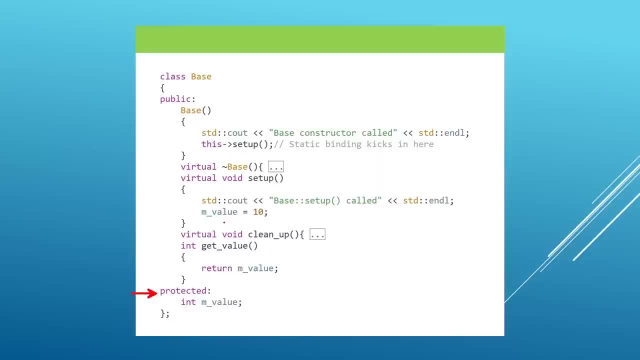 a protected member variable. it's going to have a bunch of virtual functions. we will have a virtual function to set things up and it is just going to set the value of our member variable to 10, and we're going to have a virtual function called cleanup which is going to maybe do some cleanup. 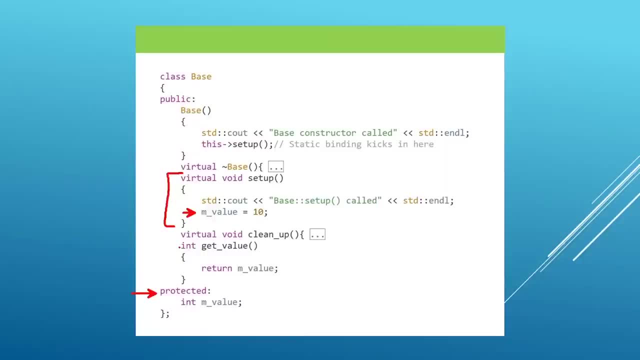 we're going to see how this works out. we also have a method to get the value, but i don't think we will use this. but you can keep that in mind and then we're going to talk about our code over here. this in, if you want. notice that we are trying to call the setup method from the constructor. 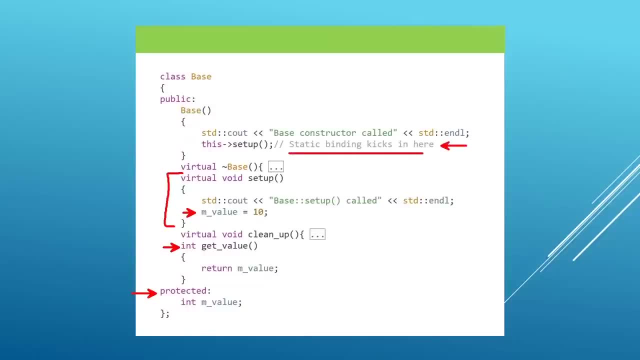 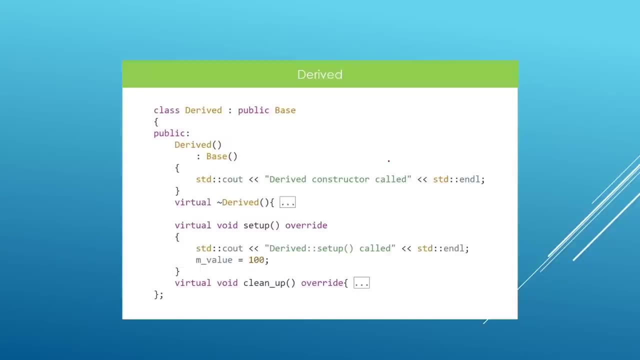 and you see that we have a comment that says that this is going to do static binding, but we're going to see why in a minute. so this is our base class. we can derive from this class and create our derived class. we're going to inherit publicly and we are going to override the methods we have in. 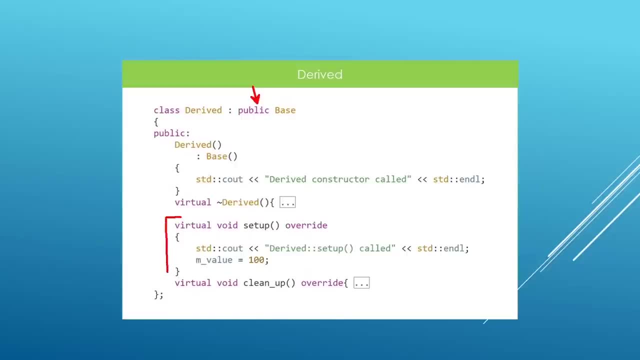 the base class. we're going to override the setup method, as you see here. we're going to override the cleanup method and our destructor is also going to be virtual, because we are good c++ citizens and this is the setup we have. once you have your inheritance hierarchy set up, you're going to 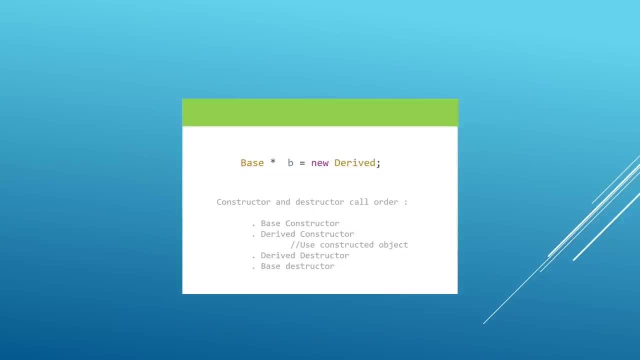 do something like this because you want polymorphic behavior. you're going to set up a base pointer and you're going to use that to manage a derived object, and you can do something like this. now, considering this statement here, i want you to think about the order in which constructors and 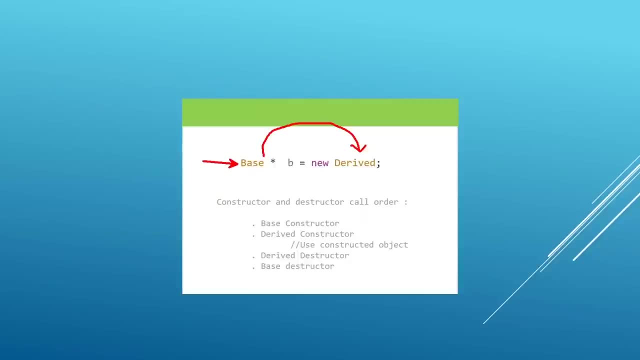 destructor are going to be called. we have touched on this subject before and we are going to revisit this because it is really important in terms of calling virtual functions in destructors and destructors. so when we do something like this, the base part of this object is going to be built first. 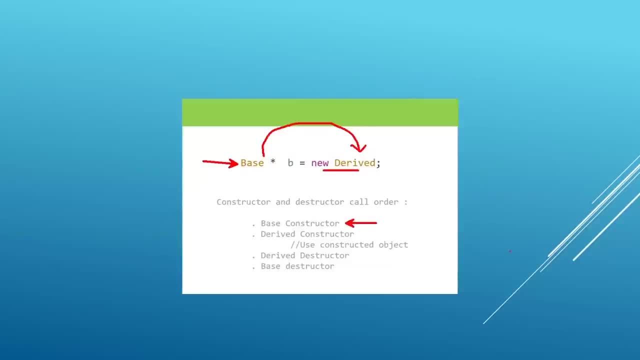 so we are going to call the base constructor first. we're going to set up the base part of us, after that we're going to set up the derived part of us and we're going to call the derived constructor. and after the derived part of us is set up, we can use our object, like we do always. so we're going to use. 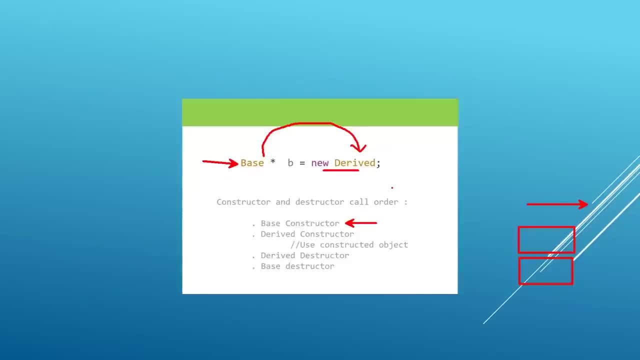 our object to do whatever it is we want to do. when the time comes for this object to be destroyed, we're going to destroy the derived part first and then we're going to destroy the base part first. now that we have considered this order, try to think about the setup when we call. 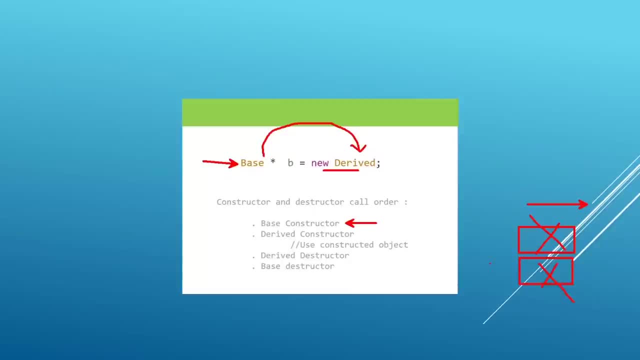 a virtual function from a constructor. that's what we're going to look at. first, the base constructor is going to be called. but notice that by the time we call the base constructor, the derived part of us won't be set up yet. so if we try to call a virtual function in the 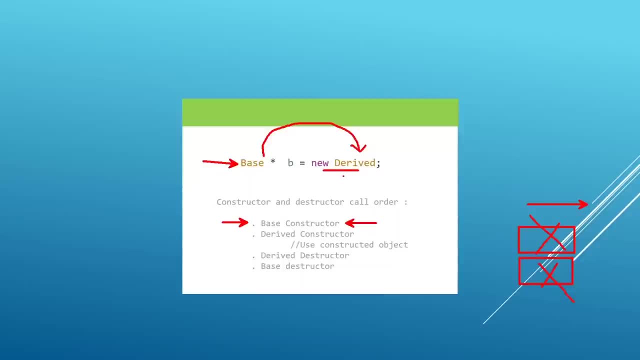 base constructor, there won't be a derived part to call the most specialized method for, so the compiler will notice that we don't have a derived part yet. we will be at this stage building the base part, and if we call a virtual polymorphic function, we want the most specific parts to be. 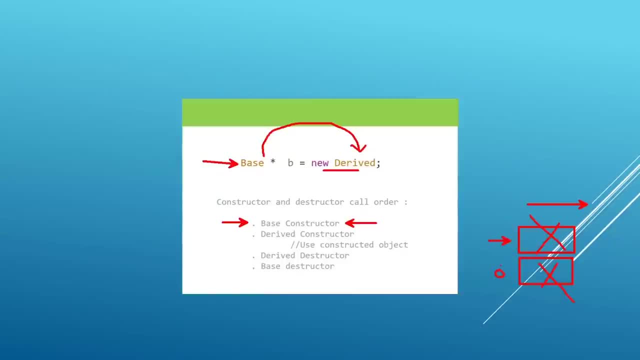 called, which should live in the derived part. but we haven't done the derived part yet. we are still building the base part of us. so the compiler is going to notice that we don't have a derived part and it is going to call the base version of our virtual function. that's why we 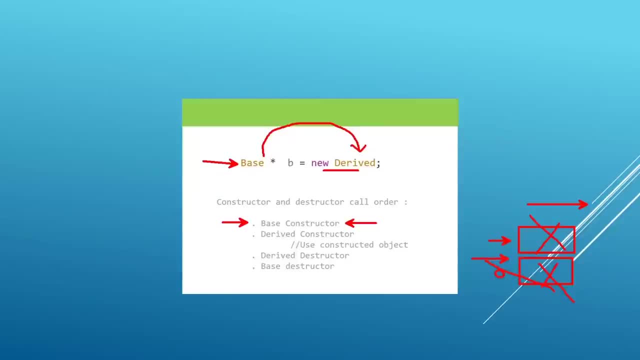 said that if you call a virtual function from a constructor or a destructor, you're going to get static, binding results. if you call a virtual function, you want the base function to be called, most specific version called. but we don't have that yet in the base part because the derived 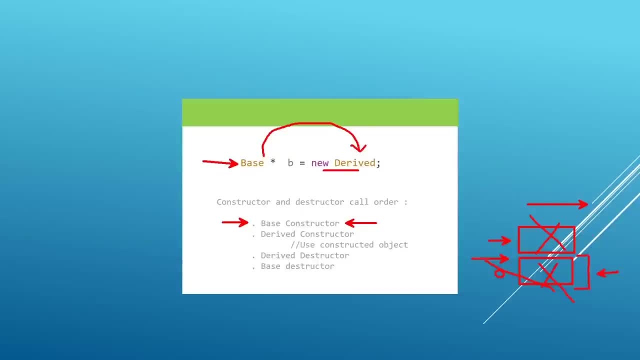 part haven't been set up. that's why we get static, binding results. i hope this makes sense and we're going to get the same result if you try to call a virtual function from a destructor. if we get to the point where our object needs to be destroyed, the derived part is going to be wiped out first. 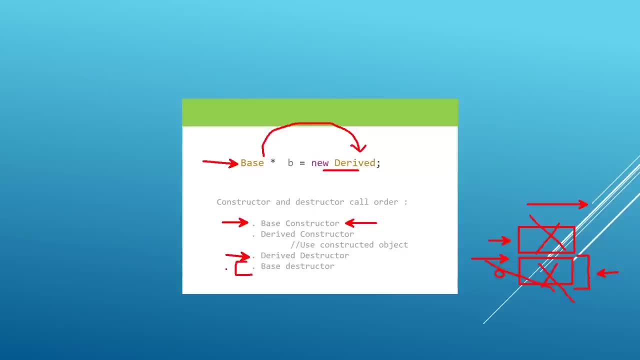 we're going to be left with a base destructor. and when we hit this base destructor and call a virtual function, that would mean to call the most specialized version of that method, but the derived part of our object has been already wiped down, so this is no longer existent and we are trying to 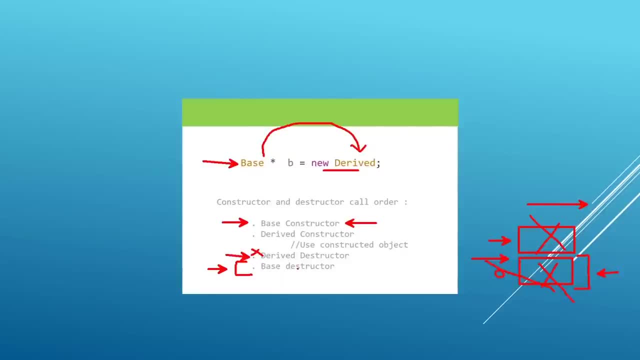 call a method on this, so the compiler is going to do the next best thing it can do. it is going to call the best version of our virtual function and again we are going to get static, binding results. that's why it isn't really wise to call a virtual function either from a constructor. 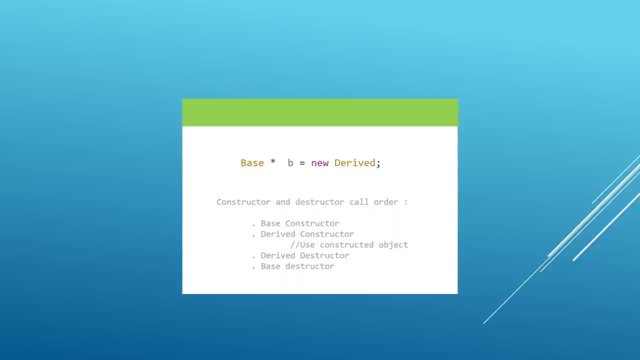 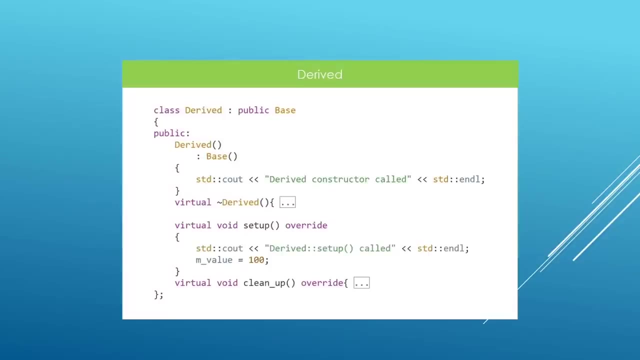 or a destructor. now some of you must be asking: what if i really need to do set up and clean up in the way that we set up these things in our classes? what if this method is really useful? maybe it is setting up things we're going to be using in our application. we really need this. 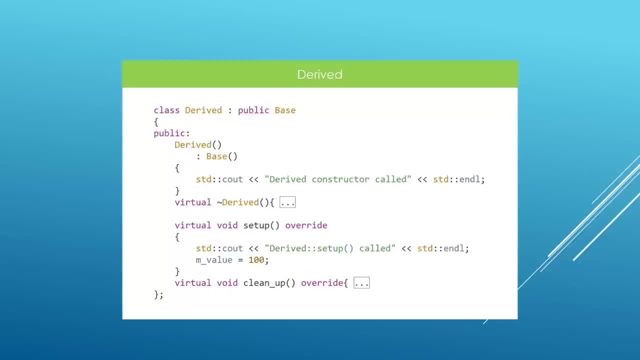 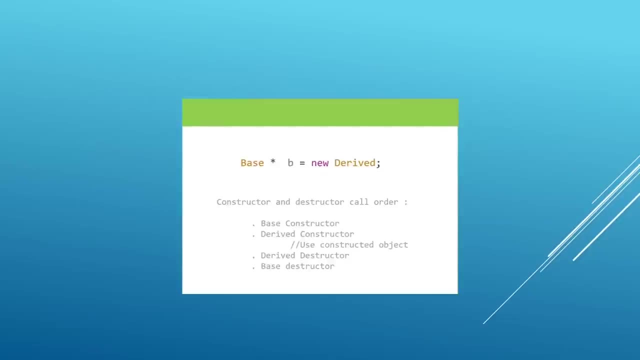 and the most logical point to call this is the base constructor. well, you shouldn't really put this in a constructor. what you could do is maybe call this virtual method on your object directly when the object has been being a constructor. That's going to be a better place to do this, because if you put that in a 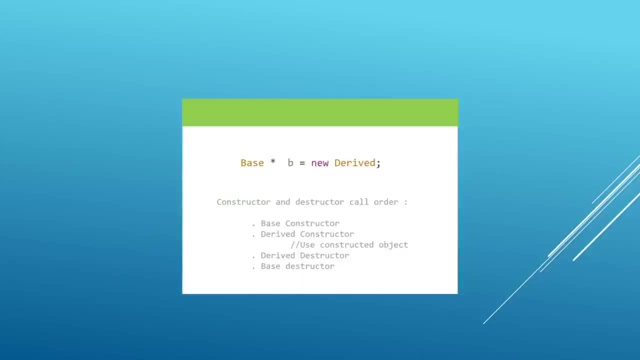 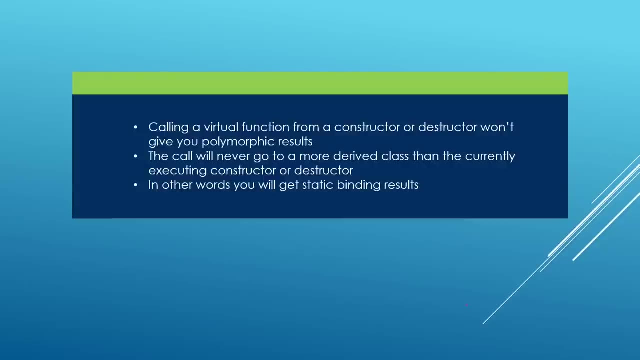 constructor or a destructor, you're not going to get dynamic binding results, and that's going to be really bad. So to sum up, calling a virtual function from a constructor or a destructor won't give you polymorphic or dynamic binding results. The call will never go to a more derived. 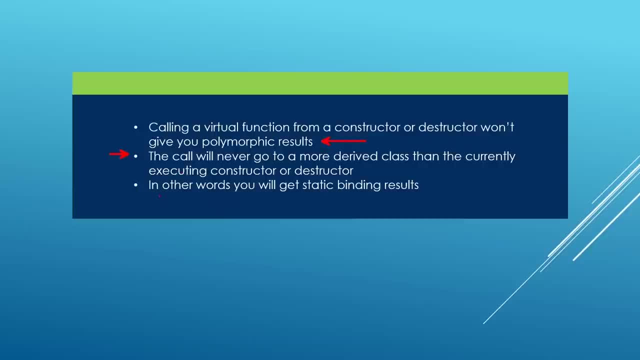 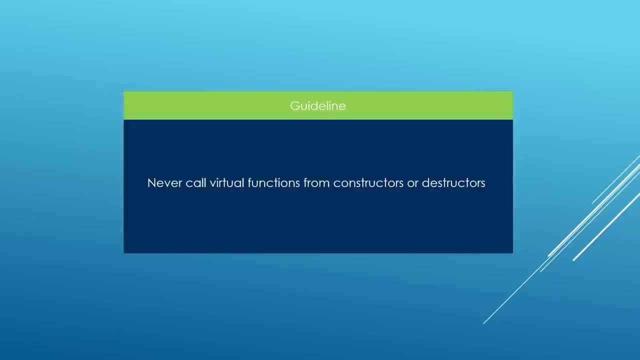 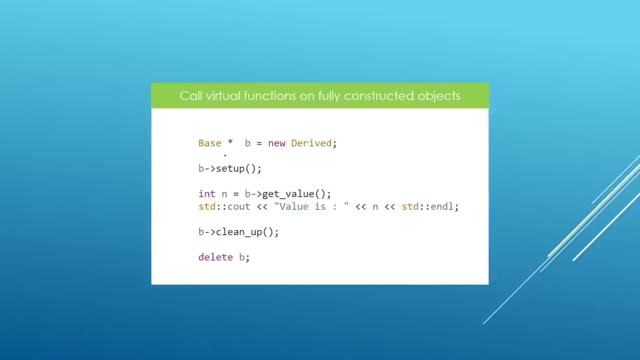 class than the currently executing constructor or destructor and we will get static, binding results. This is the idea I want to convey here and, as a guideline, you should never call virtual functions or polymorphic functions from constructors or destructors. If you really need this, the next best thing you can do is to call your virtual functions directly on your object. 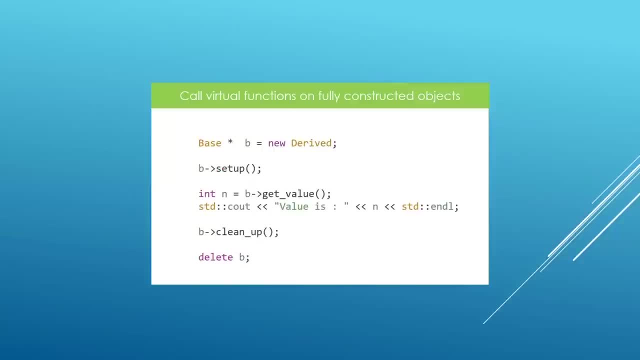 after the object has been properly set up. We can do something like this and call our setup method, and then we can call cleanup when we think that we need to clean up, and you call cleanup when you think that you need to clean up up after you construct the object and you call delete after you clean up your object. this is: 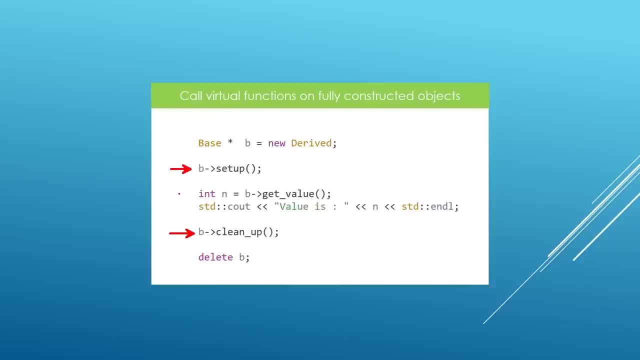 going to do whatever it is you want to do with your polymorphic functions and the calls to these virtual functions want to be living inside a constructor or a destructor, and this is going to work really well. now that you know this, we're going to head over to visual studio: code and play. 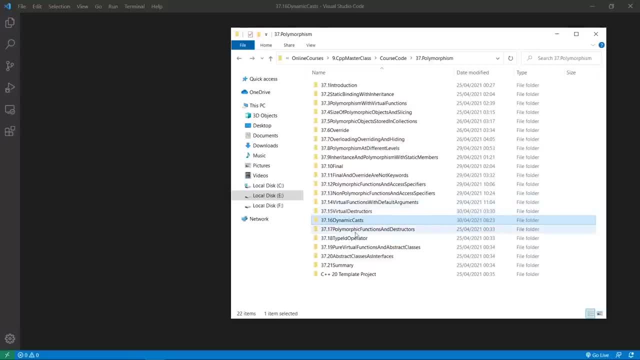 with this a little more. here we are in our working folder. the current project is polymorphic functions and the destructors. we should really say with constructors and destructors. but this is going to do. we're going to grab our template files and we're going to put them in place and we are going 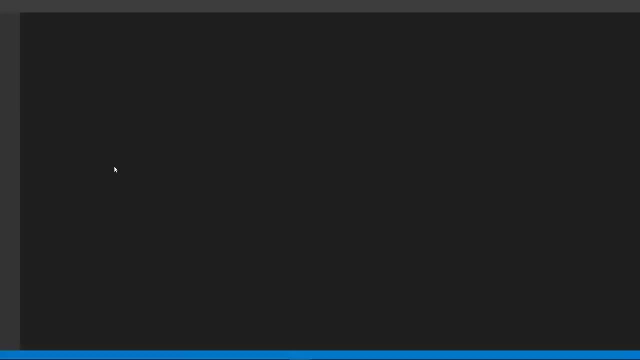 to open this little guy in visual studio code by dragging and dropping here. this is going to give us our main cpp file. we can clean up a little bit, remove whatever it is we don't need, and i am just going to put in my classes. i am going to do that in the main cpp file because that's going to be. 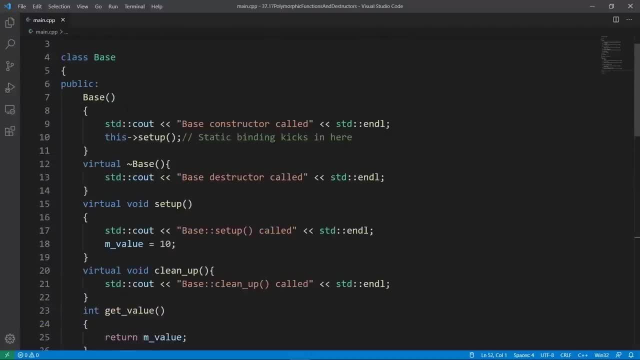 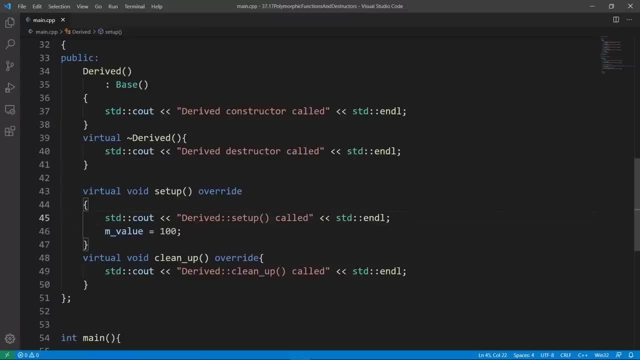 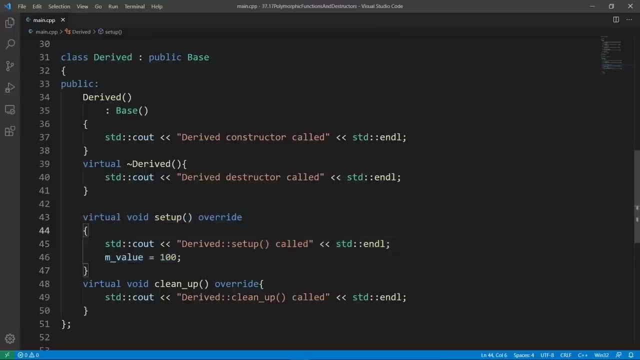 own member variable. all it's going to do is set up a bunch of overrides for the virtual functions we have in the base class. we're going to override setup and in derived we're going to set our value to 100 and we're going to clean up and put a message that we are cleaning up here once we 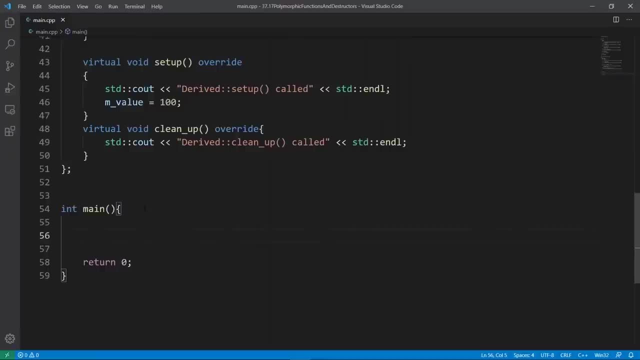 have this set up. we can head over in the main function and set up a base pointer which is going to be managing a derived object, a classic setup for polymorphic behavior. so we're going to say base and i'm going to say p base and we're going to say equals new derived. this is going to give. 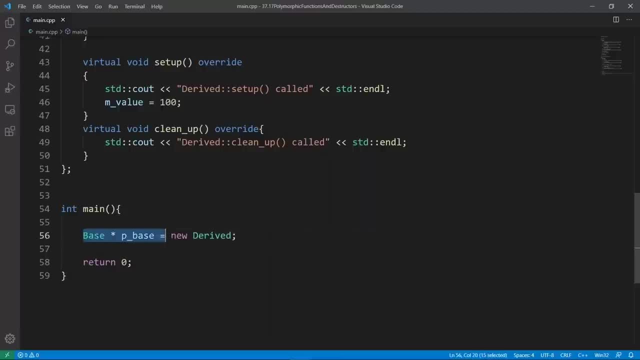 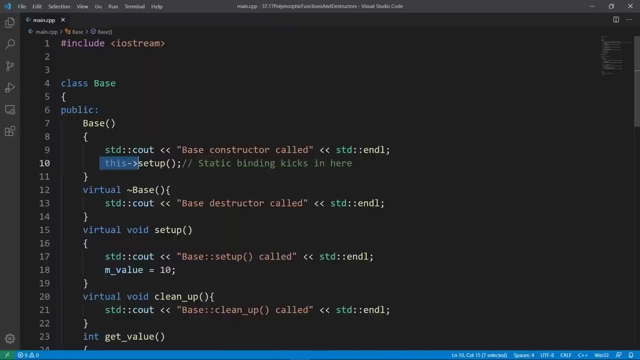 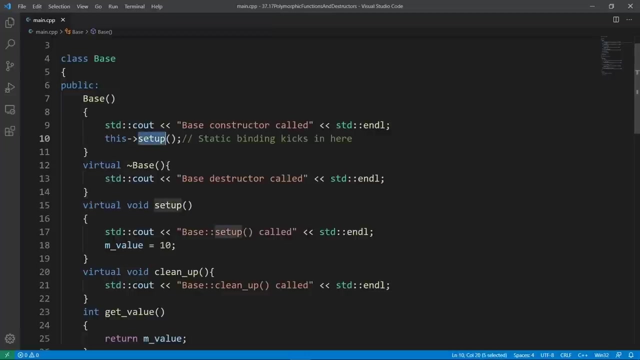 us our object, which is managed by a base pointer. and one thing i didn't show you is that we are calling the setup virtual function from the base constructor. this is what we want to see. we want to see what is happening here now. if we call this setup function, we would expect 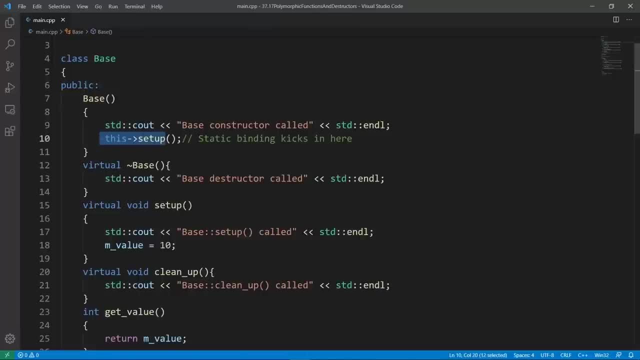 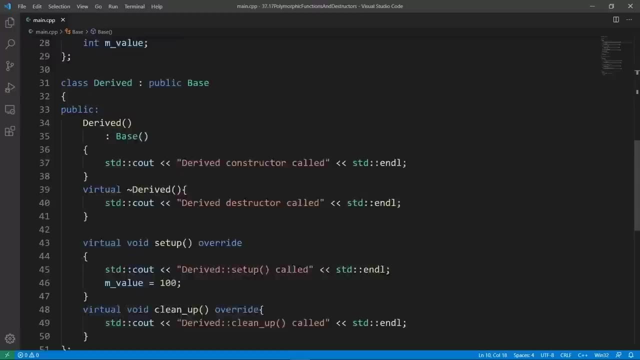 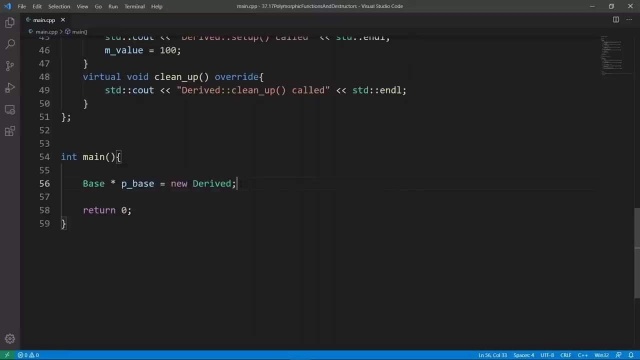 polymorphism to kick in, because this is a virtual function. if the derived part is available, we will call the most specific setup function and that would set up the value to be 100. here, if we get the value, that's what we would get. let's see what we get here if we try to get the value. 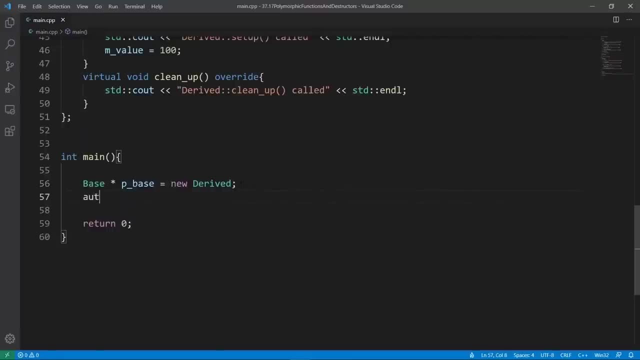 that we have in this object here. so we will get auto value and we're going to say p base, get value. we have this function here and we will try to print this out. okay, this is something we can do in our c plus plus program and we're going to see the value we get because we are 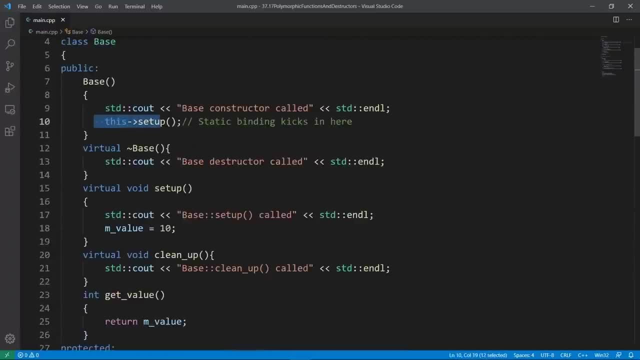 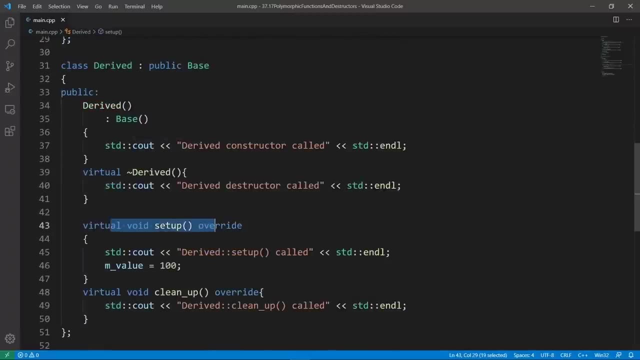 calling this virtual function, we expect polymorphism to kick in, and if polymorphism kicks in we're going to call the most specialized version of our virtual function here. that would be the override we have in derived and that would give us 100, so one would get to get 100 printed. 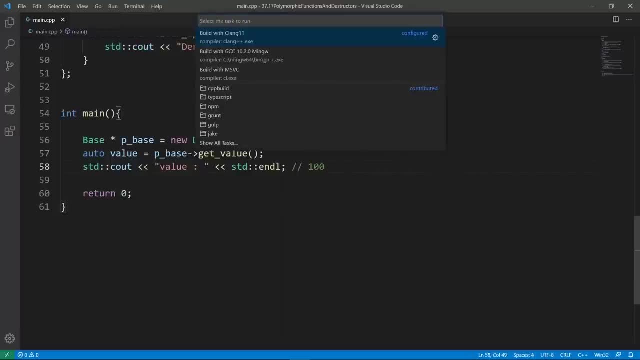 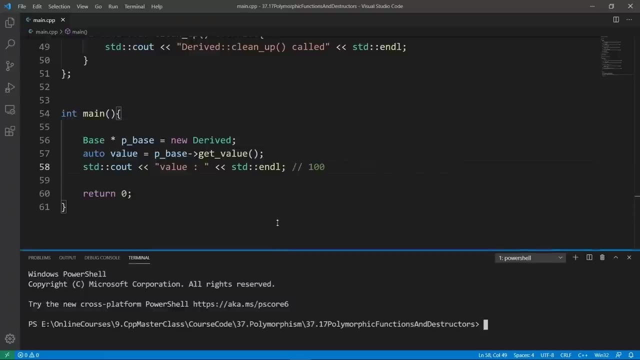 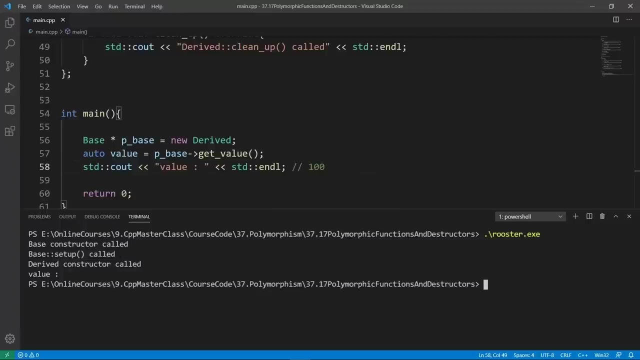 out here. but let's see what we get. we're going to run this through gcc, our favorite compiler. the build is going to be good. we can clear or bring up a powershell window. we're going to clear now and run rooster. we're going to see that the base constructor is going to be called. base setup was called, you see. 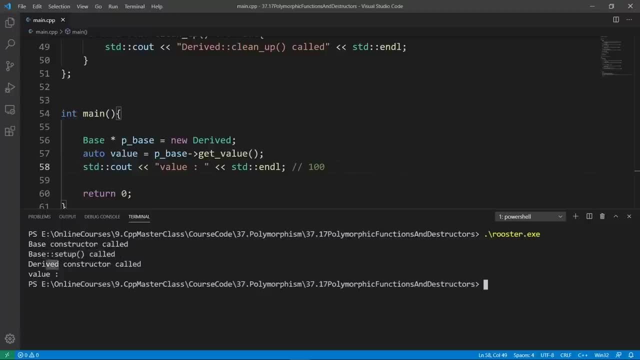 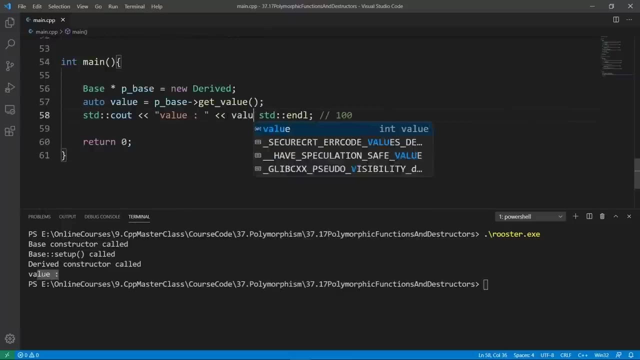 we call the base version of this and the derived constructor will be called, and we're going to see that the value doesn't exist. oh, we didn't put the value out. let's do that, my bad. here we're going to build again. we're going to use gcc to bolt and the build is good. we can clear and run. 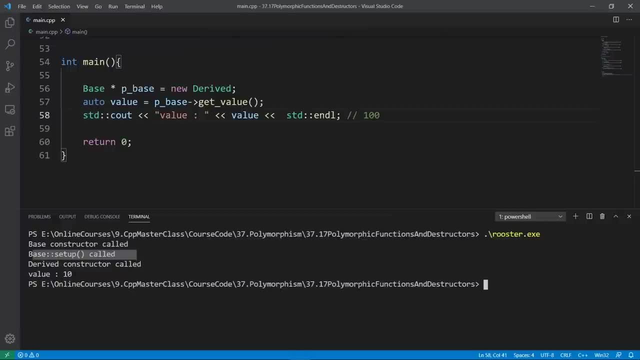 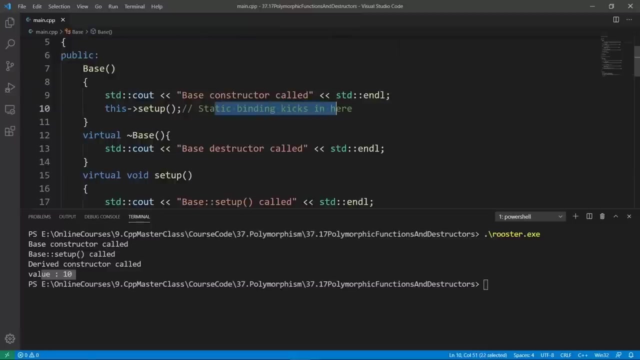 rooster. now we see that the base setup method was called and set the value to be tan and we are really getting static binding results because we are calling the setup method from the base class and the base version is being called. so this is classic static binding behavior, but we want polymorphic behavior. 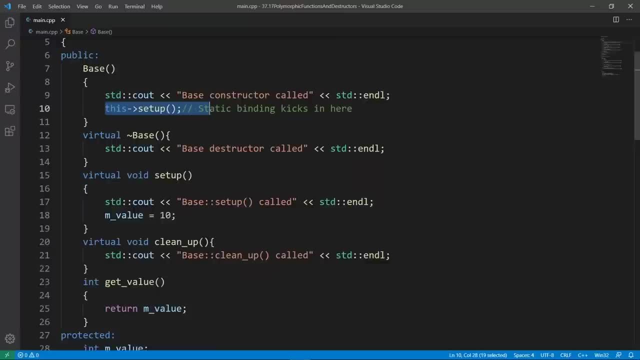 to be working here, but we just saw the reason why this is in the slides by the time we call this virtual function. we haven't set up the derived part of us yet and we have no way to call this virtual function, which means that we're going to call this virtual function, which means that we're 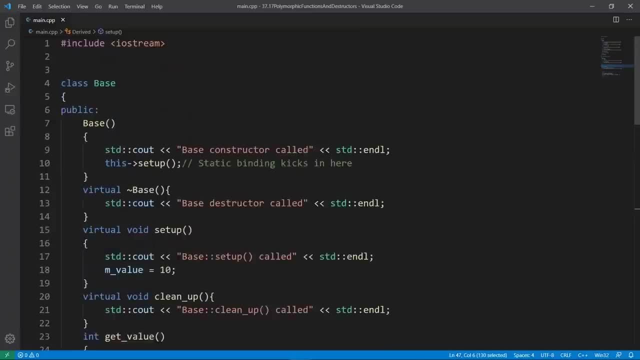 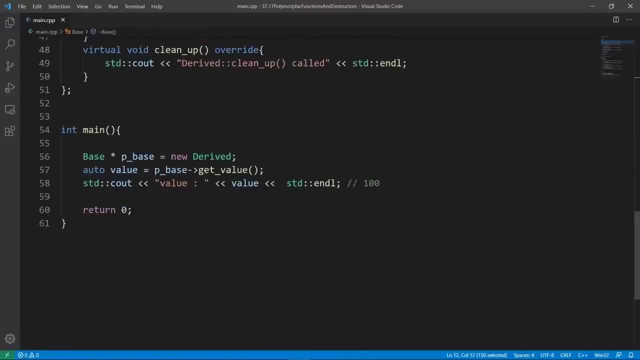 going to call this virtual function which leaves in the derived part of us. so the compiler is going to do the next best thing it can do: it's going to call the base version of this method and we are going to get static, binding results. and we are going to get the same results if we 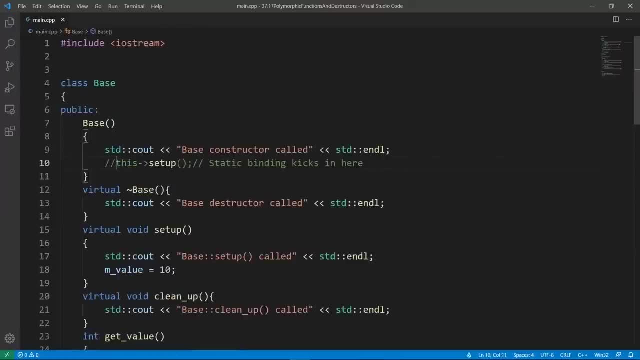 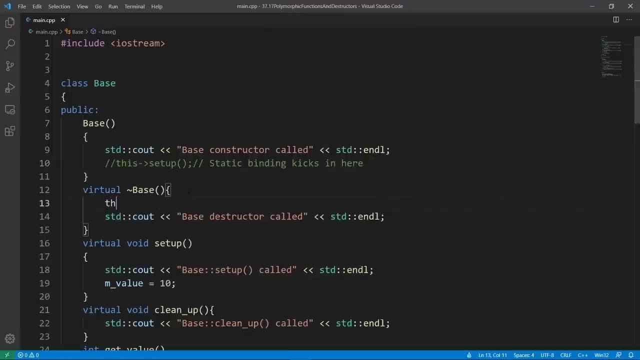 try to call a virtual function from the destructor. for example, if we go in our destructor here, let's see if we can find it. we're going to go in our destructor here and say this and say cleanup. you can do something like this and you're going to see that the cleanup version 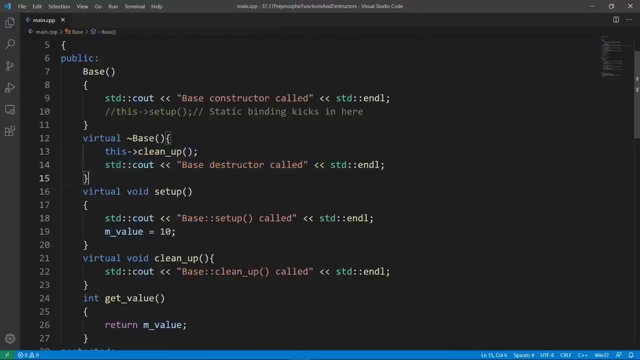 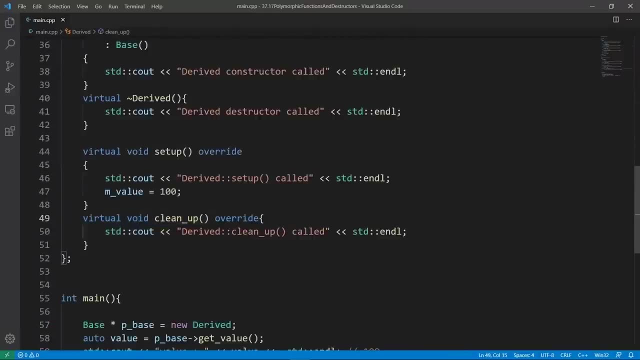 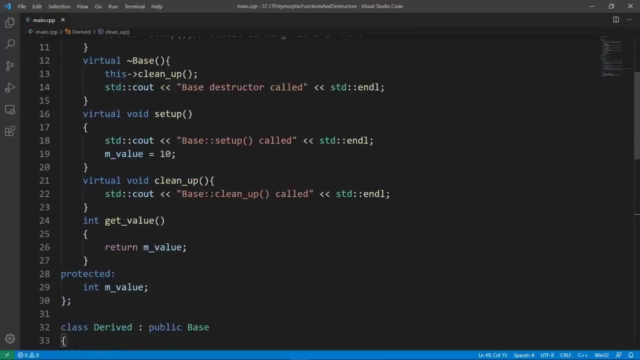 we call is the base version of cleanup, and we don't really want to do something like this. we want the most derived cleanup version to be called, but we won't get that because by the moment we call this virtual function from our base class, the derived part will already have been wiped out. 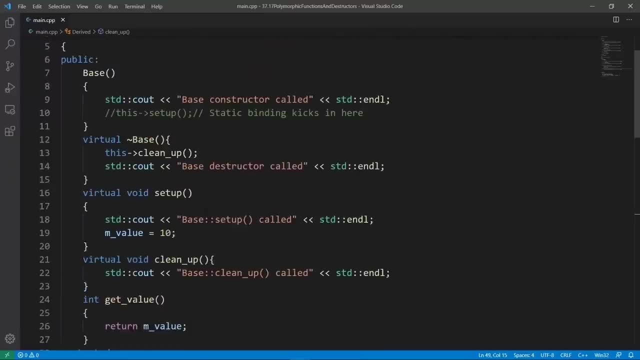 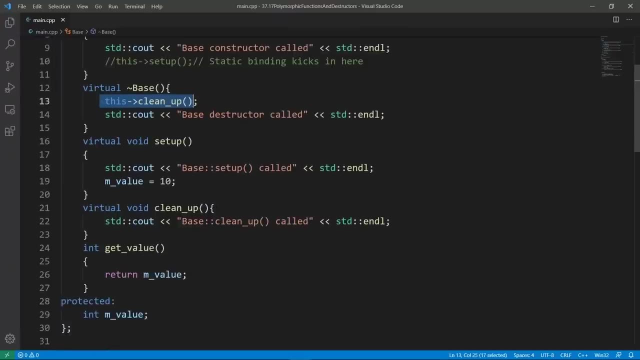 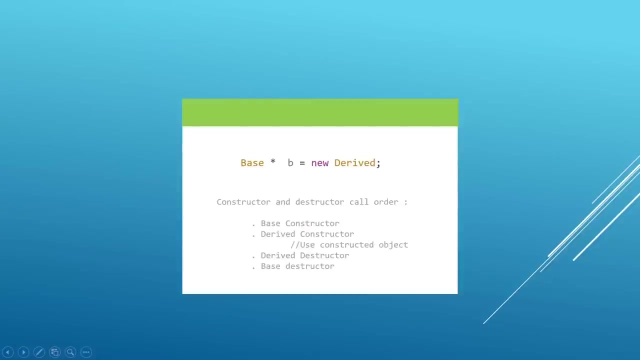 so it won't be available and the compiler will do the next best thing it can do. it is going to call the best version of our cleanup function here. i hope this makes sense again to really drive this home. i realize this can be confusing to many people, especially beginners, if we are calling a virtual function from a constructor. 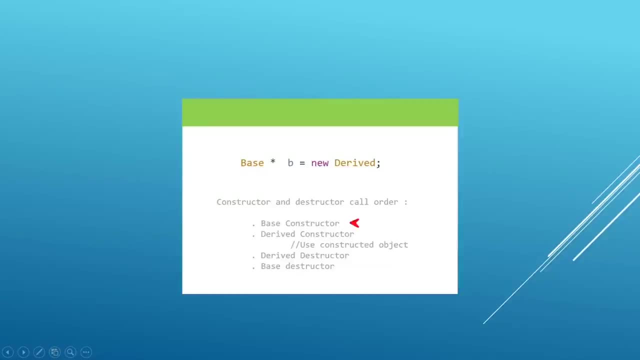 we will call that original function when we hit the base constructor. but by the time we hit the base constructor the derived part of us hasn't been constructed yet. so if we try to call a polymorphic function, needing to call the derived implementation, that won't be available and the compiler will do the next best plan it can do. it is. 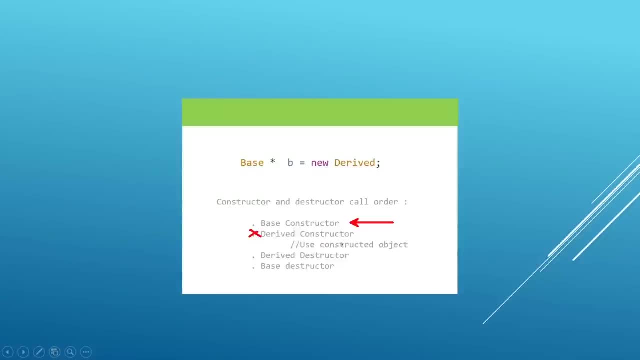 going to call the base version. the same phenomenon is going to happen in the destructor. when we are done using our object, we will destroy the derived part information first, and when we hit the base destructor and call a virtual function, there won't be a most specialized version of the virtual. 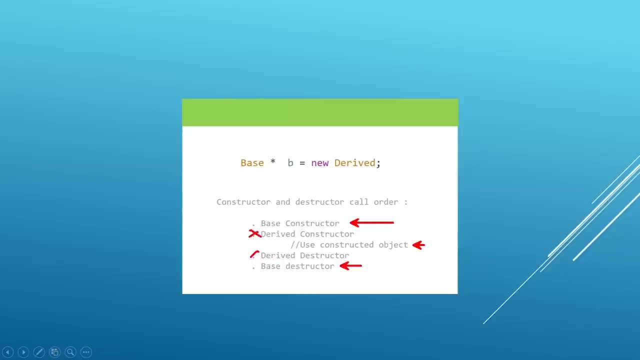 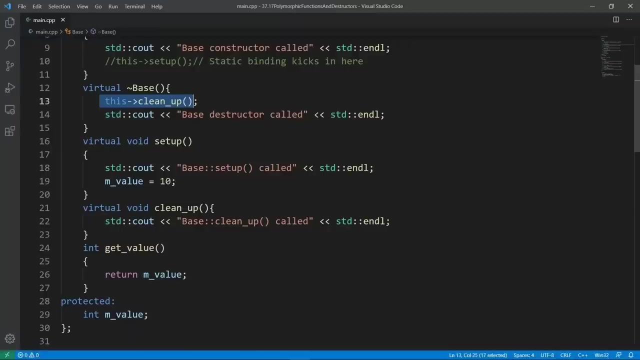 function because the derived part has been already destroyed and it doesn't exist anymore. so if we call a virtual function from the base destructor, we will get the best version called and this will give us static, binding behavior. this is what we are experiencing here. okay, so let's try and run. 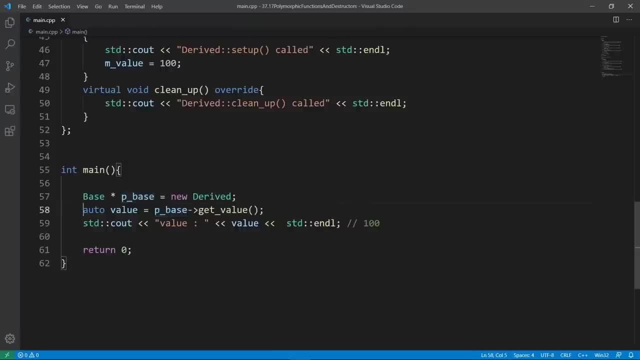 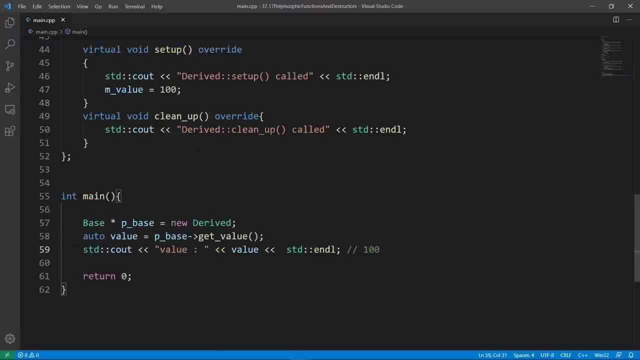 this program and see what we get. we will print our value here, which is going to give us static, binding results, but we want to see which version of cleanup is called. this is what we want to see here. we're going to run the task to build with gcc. the build is going to be good as usual. we're going to 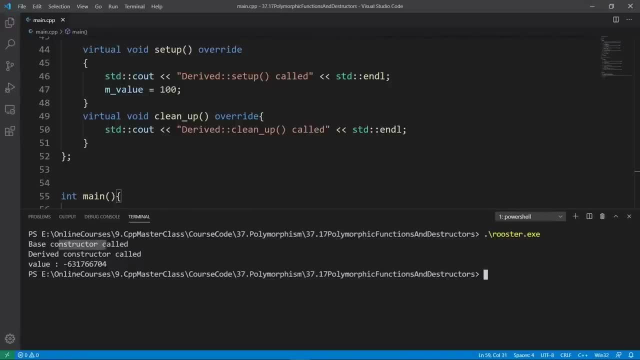 clear and run rooster and we're going to see base constructor called derived constructor called and we're going to run the task to build with gcc. the build is going to be good as usual. we're going to clear and run rooster and we're going to see base constructor called derived constructor called and we're going to see base constructor called derived constructor called and we're going to 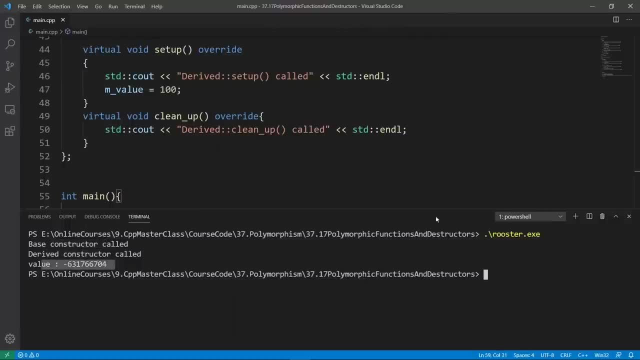 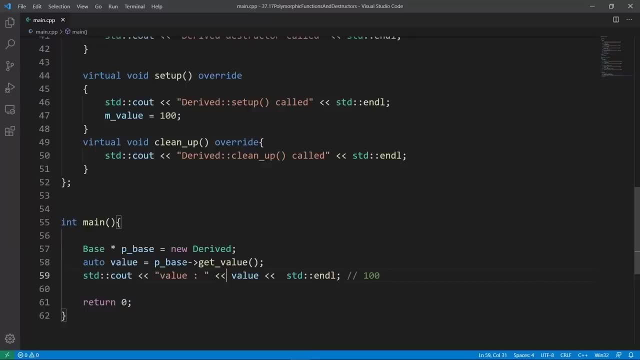 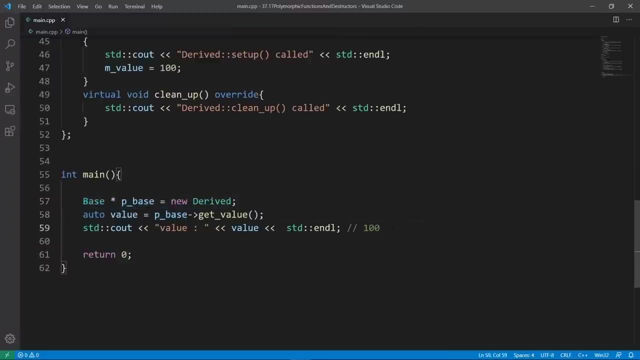 have a value which is a junk value because we never initialize this value, but we don't see our destructor is called. what is going on here? let's investigate this a little more. the reason is we are not explicitly releasing this memory here through the base pointer. let's do that. we're. 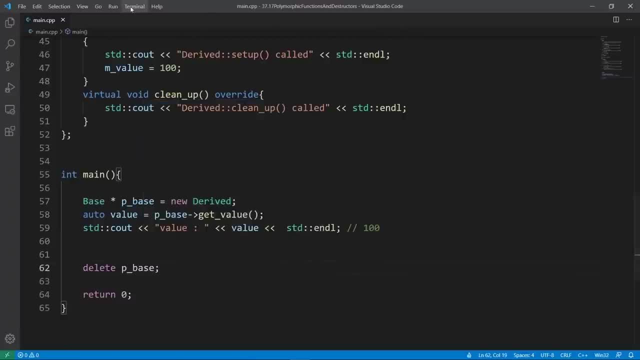 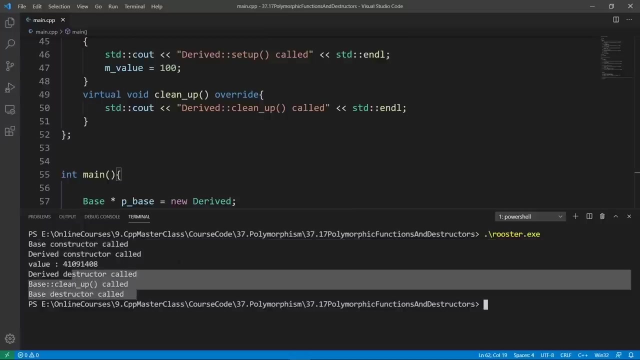 going to delete p base here and we're going to run again. we're going to build with gcc- now our destructors should be called. we're going to run rooster and we are going to see that the base clean up version was called and again this is giving us static, binding results. you don't want something. 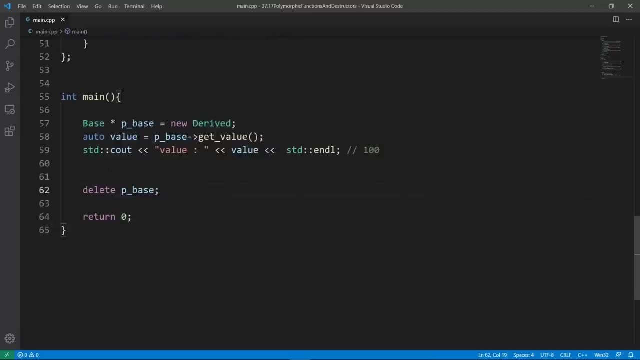 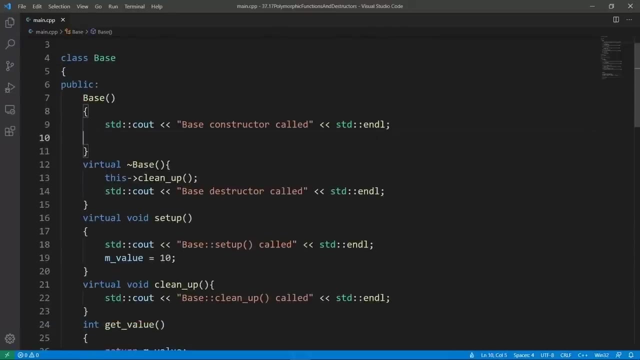 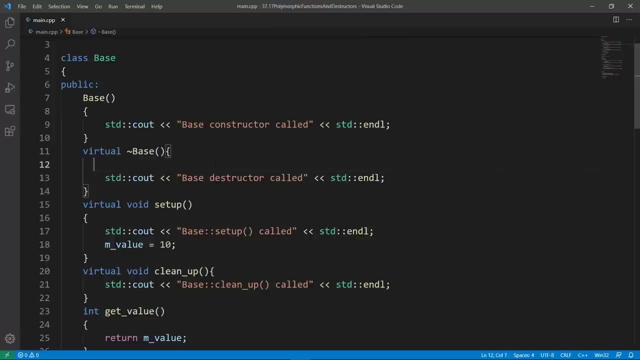 like this. so if you want to get this behavior, i would advise not to call the cleanup or setup functions inside constructors or destructors, and that's the guideline i gave in the slides. you should really never call virtual functions, either from constructors or destructors, especially if you are doing this from a parent class hoping to get the most specific. 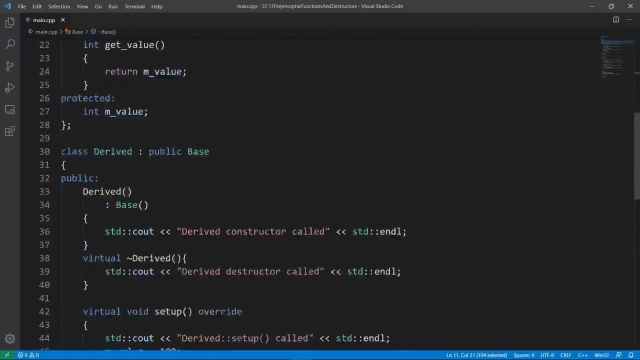 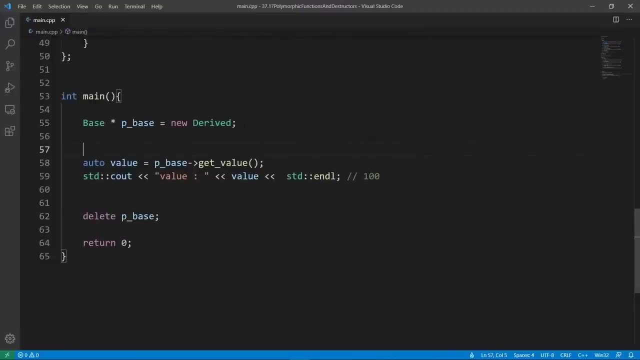 virtual function called through polymorphism. if you want to do that, the best thing you can do is to call the cleanup functions and is to call the setup and cleanup functions after your object has been properly constructed or before your object gets to be destroyed. so what you can do, 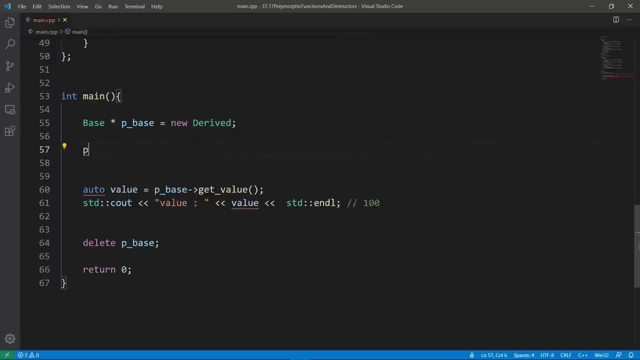 here is: call the setup method on the p base pointer here. let's do that and we're going to call setup. this is going to call our virtual function and we are going to call the setup protocol. and then we are going to do the cleanup function and we are going to call the setup. 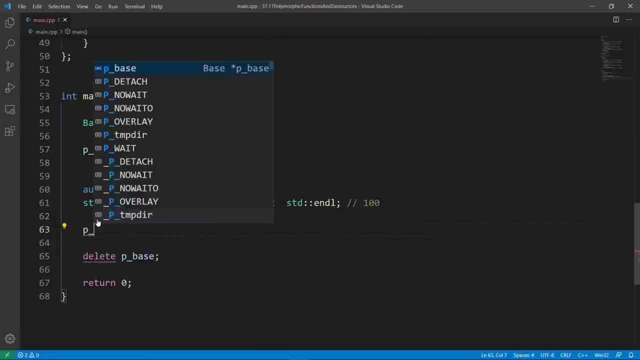 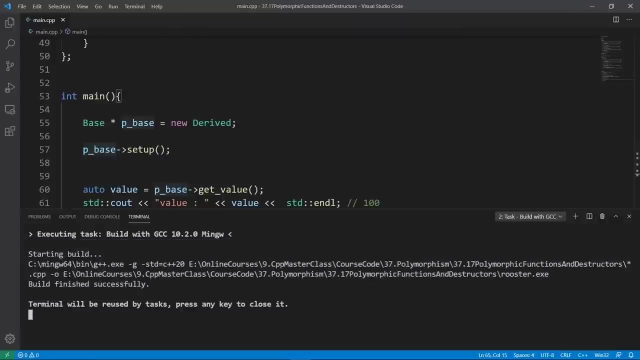 function and we're going to call the cleanup function if we need to do some custom cleanup here. so i'm going to say base and call the cleanup function and this is going to give us the behavior we want. we're going to build our program, pass this through gcc. the build is going to be good. 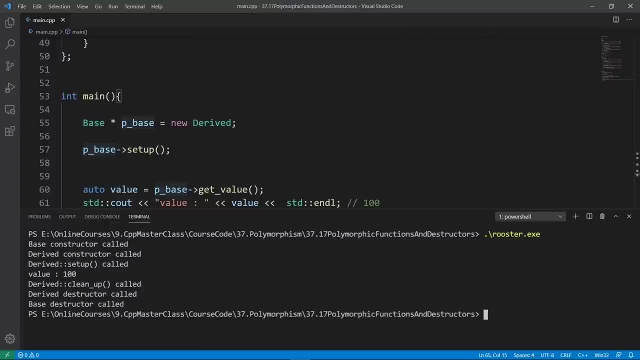 clear and run rooster and we are going to see that base constructor was called, derived constructor was called. we will call the derived version of setup. our value will be 100 and when we get to release or clean up our memory, the derived version of cleanup will be called. and then we will destroy. 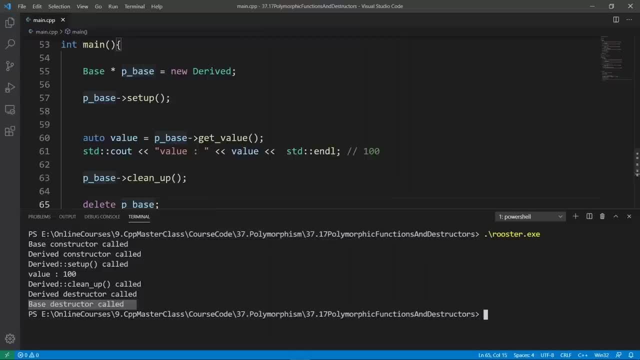 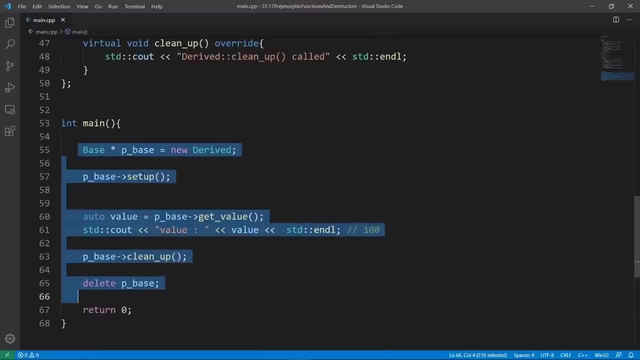 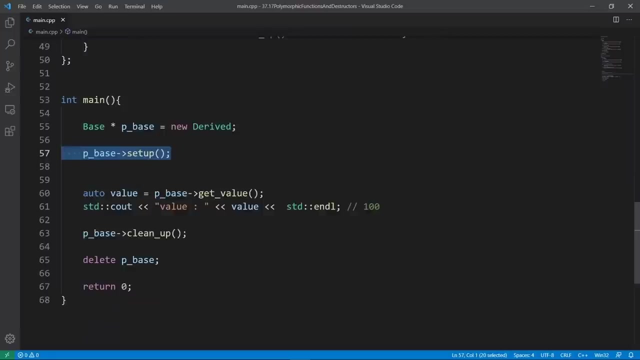 the derived part of us and then we will destroy the base part of us. this is going to work in line with the behavior we are familiar with with polymorphism, and this is really cool. so this is what you should do: you should never call virtual functions from disruptors and constructors, because 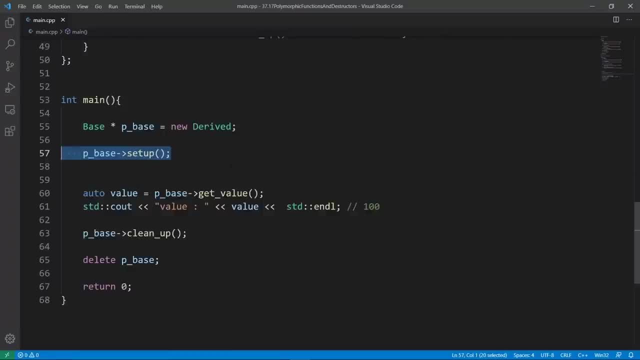 that's going to give you static, binding results, and what you want in this case is really dynamic binding behavior. this is really all i had to share in this lecture. i hope you found it interesting. we are going to stop here in this one. in the next one we're going to learn about the type id. 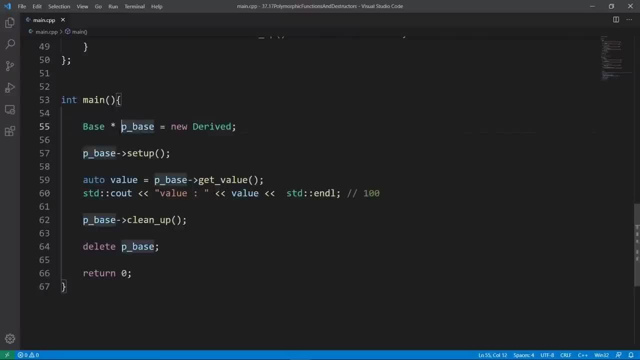 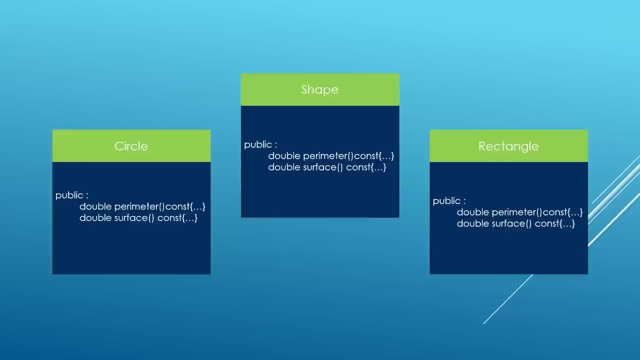 operator. that can come in handy, especially if you want to debug polymorphic code in your C++ program. Go ahead and finish up here and meet me there. In this lecture we're going to learn about pure virtual functions and abstract classes, And pure virtual functions are a mechanism we have in C++ to mean that the method 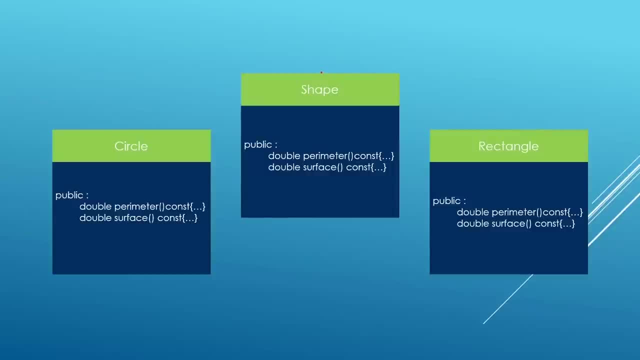 isn't meant to be implemented in the base class. Here we have a simple inheritance hierarchy to try and drive this home. The base class is shape and we are deriving from this class to create a circle class and on the other side we are deriving to create a rectangle class. If we look in the shape class, we have 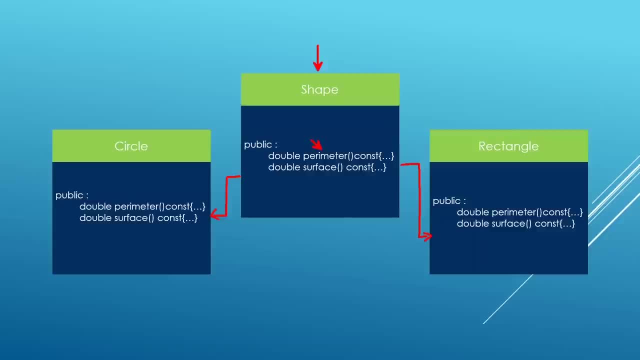 two virtual methods. One is going to be used to compute the perimeter of the shape, The other is going to be used to compute the surface of the shape. But if we go down in our inheritance classes we're going to see that we have the same. 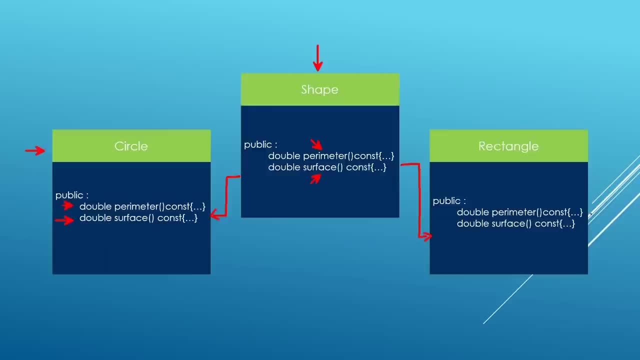 methods. These are going to be overrides of one and the same methods, So we're going to see that we have the same methods, what we have in the base class, But the special thing about this inheritance hierarchy is that we don't have implementations for these methods in the 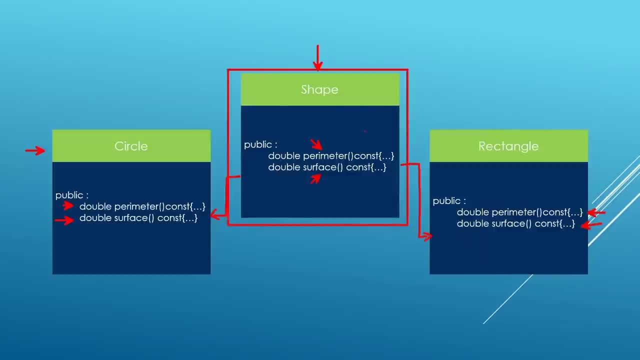 base class here And this is by design. If you think about it, this is an abstract shape. We don't know if it's a rectangle, We don't know if it's a circle, We don't know if it is a triangle. So we don't really have concrete information we can. 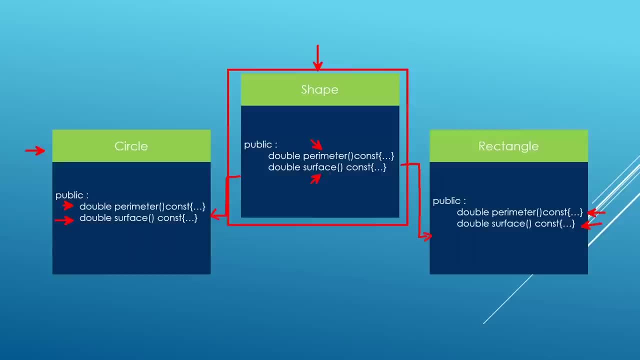 use to properly compute its perimeter and its surface. So it makes sense to really look at it from this perspective. So we leave in the declaration for these methods but leave the implementation details to inheriting classes, because these classes are going to have concrete information we can use to reliably compute the perimeter and the surface. 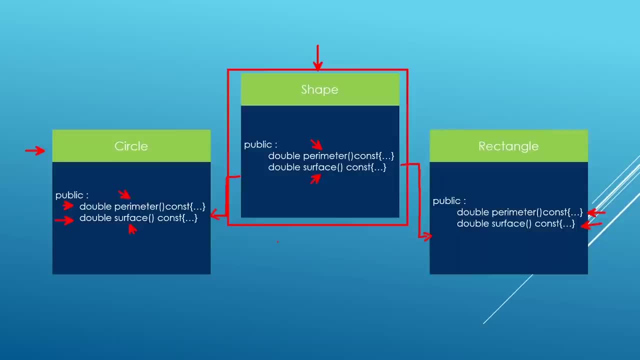 and we can get this information here. So in C++ we mean this kind of design by setting up these methods as pure virtual functions, And what this is going to tell the compiler is: these methods are not meant to be implemented In the base class. they are meant to be overridden and implemented by 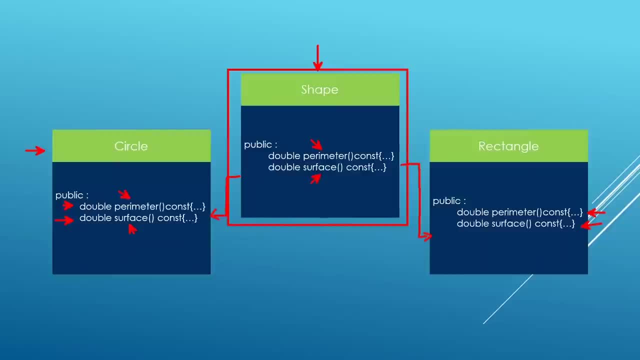 inheriting classes, And another side effect of this is that the compiler is going to prevent you from creating objects of these class, because it really doesn't make sense to create an object of shape in your design if you won't be able to compute its perimeter, if you won't be able to compute its surface. So 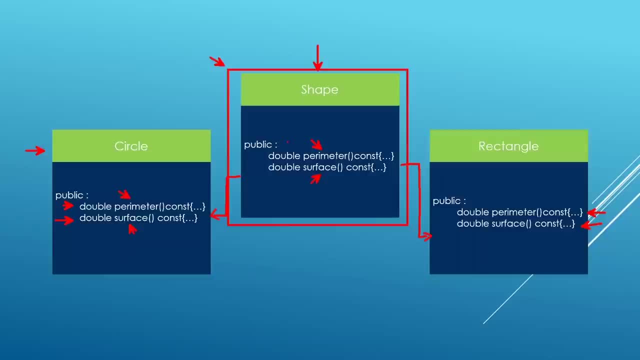 why bother creating an object that you won't really be using in your C++ program So we can use this base class just to be an idea or a representation of a shape, without really going into the concrete implementation of how that shape really works? Hopefully this makes sense. So let's see how we can do this in code. 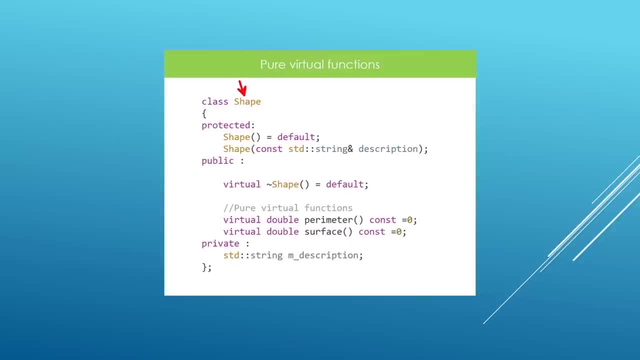 Here we have a simple class which is going to be our shape class. We are going to have two virtual functions. We're going to have the perimeter function, We're going to have the surface function. These are going to be virtual functions or virtual member. 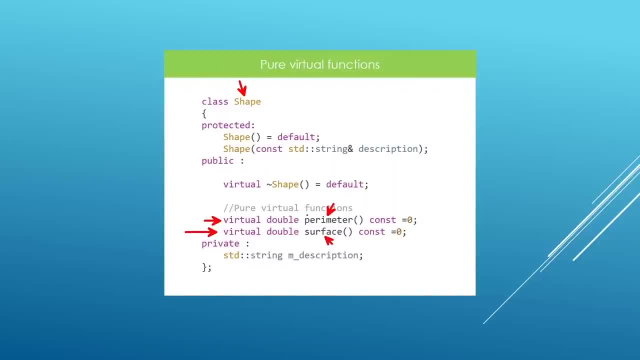 functions, I should say, But we are going to make them pure virtual functions by using the syntax you see here. So we're going to prepend an equals zero and this is going to tell the compiler that these are pure virtual functions. Once you set up these, 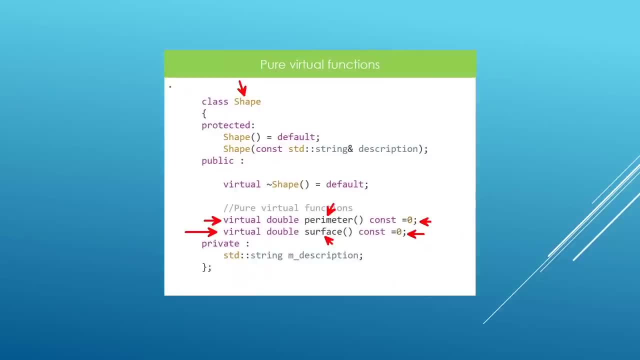 functions. a few things are going to happen in your class. This class is going to become an abstract class, in that you won't be able to create objects of this class anymore. If you try to do that, you will get a compiler error. Another thing is that you don't need to put in implementations for these methods, because you 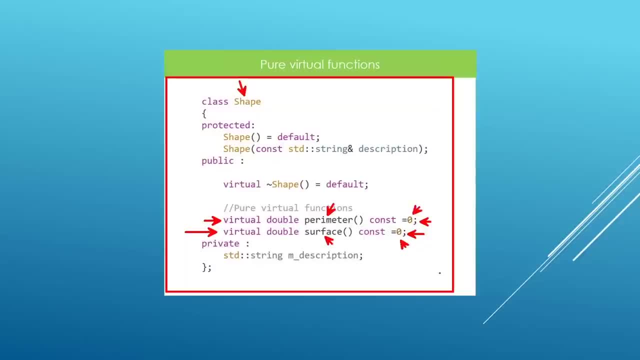 marked them as pure virtual, And what this means is that the implementations will be put in by inheriting downstream classes, because they will have concrete information to compute the perimeter or the surface, as we have here, So we don't need to bother with definitions for these. 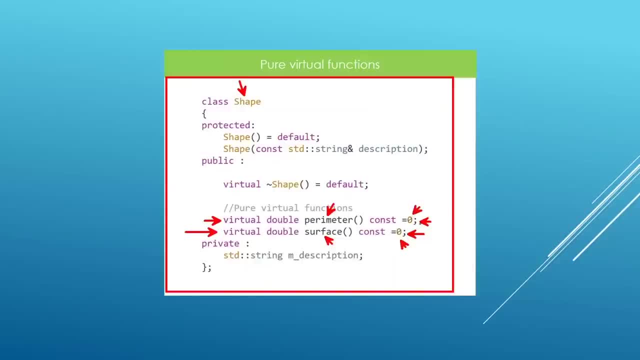 functions here. If you even try to put in a definition here, you're going to get a compiler error because this is a virtual function. We have no business putting an implementation in the base class here. These are meant to be implemented by downstream inheriting classes. 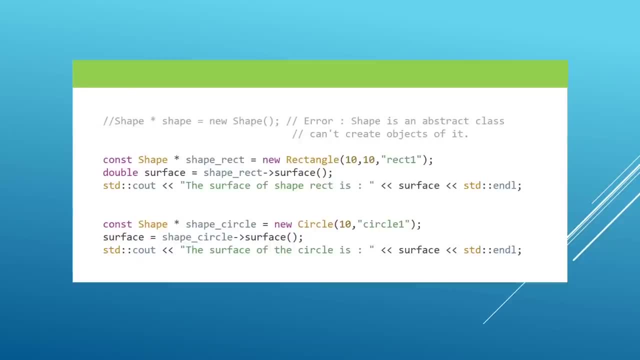 OK, Once we have our shape class and our inheritance hierarchy, we can try to run this in our code. For example, if we try and create a shape object, we're going to get a compiler error because the shape is an abstract class, so we can't create objects of it, And I don't think I made this super clear. 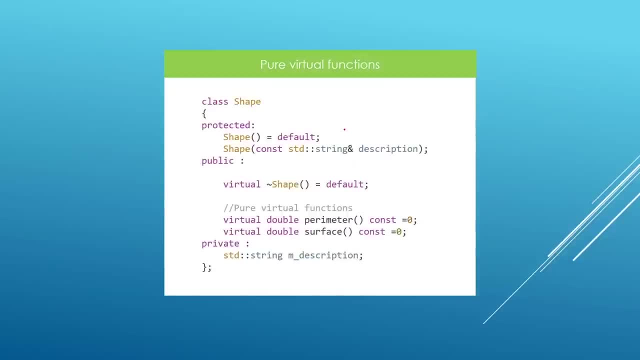 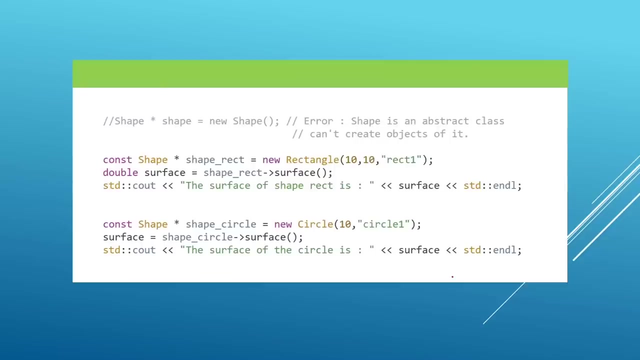 Once you set up at least one pure virtual function in your class, the class is automatically going to become an abstract class, And what that means is that you want to be able to create objects of this class. So this is an abstract class we have here, And if we try to create an object of it, as we are doing, 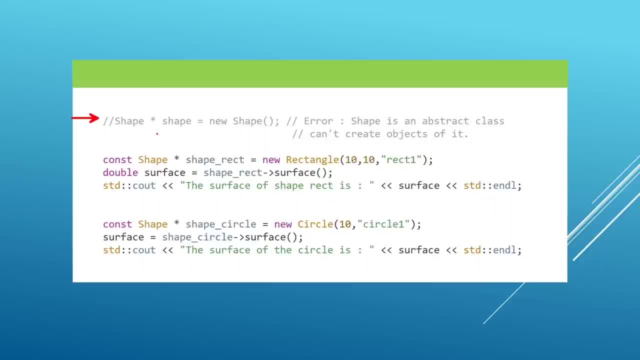 on this line. here this is going to give us a compiler error, But we can still use a base pointer to manage a derived object, a common setup. we do with polymorphism. So for example, here we can set up a shape pointer and use this to manage a rectangle. 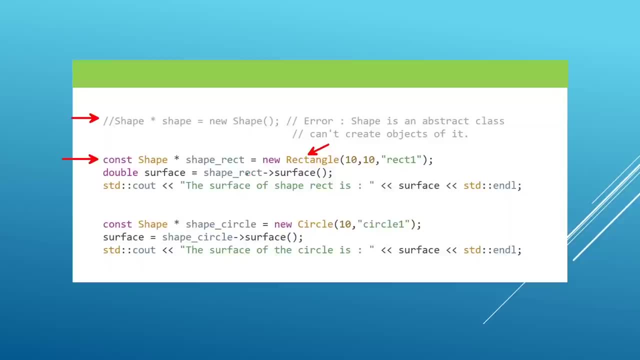 object. If we call the surface member function on our base pointer, this is going to do a polymorphic call and we will get to the surface of the rectangle And we're going to print this out here. You're going to see that this is going to work. 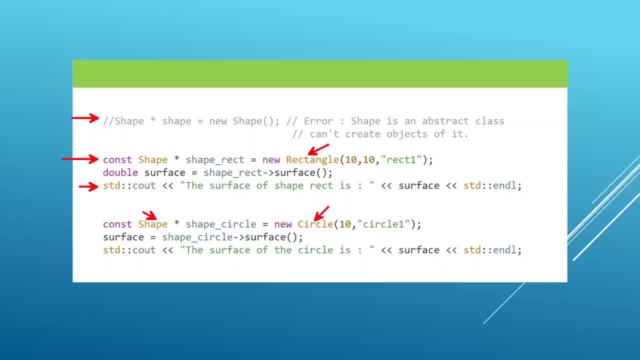 We can also use the base pointer to manage a circle object. as we see here. If we call the surface method, this is going to do polymorphism and it is going to call the surface version of the circle class and we can see it printed out here. 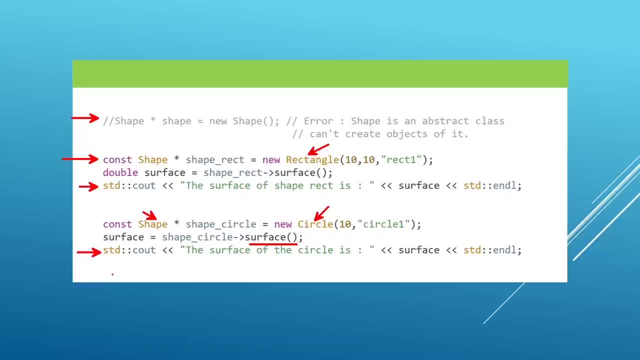 This is the design we can achieve, Even if shape is an abstract class. we can't create direct objects of shape, as we are doing here, but we can use a base pointer or a shape pointer to manage derived object through polymorphism, and you need to be aware of this. 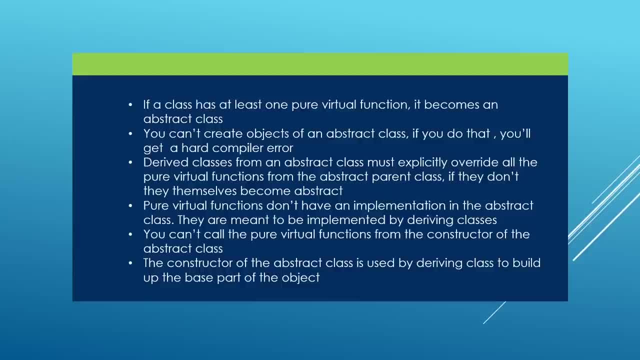 Okay, now that you have an idea about what a pure virtual function is and what an abstract class is, Let's see a few ideas you need to keep in mind. If a class has at least one pure virtual function, it will become an abstract class. 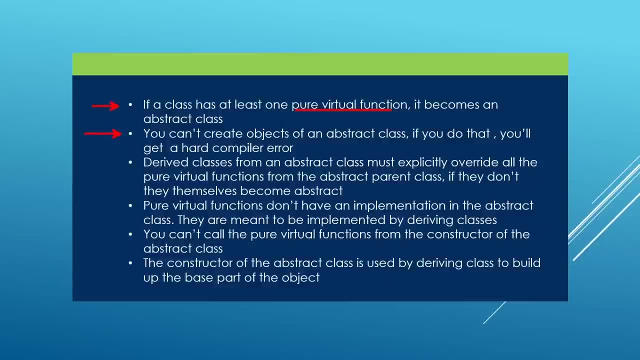 You already know this: You can't create objects of an abstract class. If you try to do that, you will get a compiler error. Another thing I don't think I made super clear is that derived classes from an abstract class must explicitly override all the pure virtual functions from the base class. 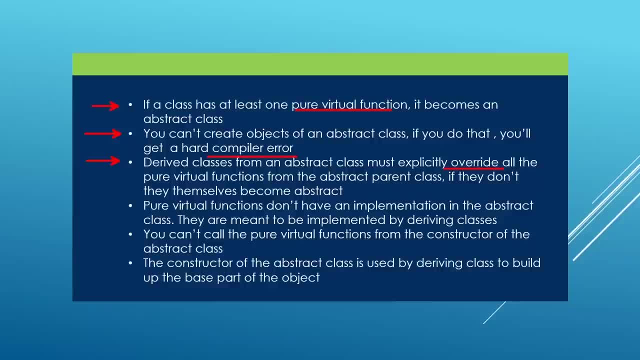 If you leave in any of these classes, you will get a compiler error. If you leave in any of these classes, you will get a compiler error. If you leave in any of these classes, you will get a compiler error. Any pure virtual class that you don't put in an implementation in for your derived class. 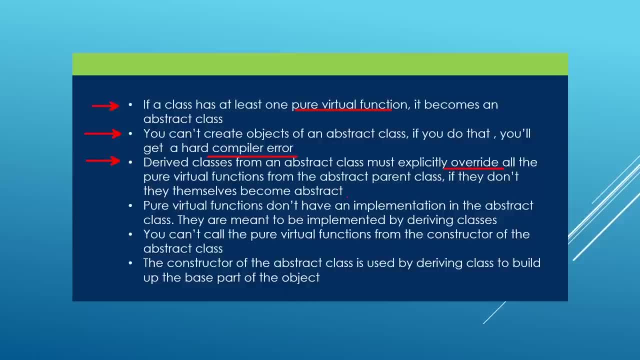 is also going to become an abstract class and you won't be able to create objects of it. You need to keep this in mind. Another thing you can't do: you can't call the pure virtual functions from the constructor of the abstract class. 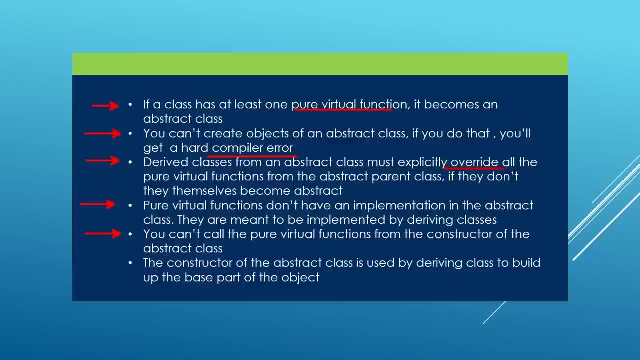 If you do this, you're going to get a compiler error because we don't have implementations for these things, So this is not going to work. The constructor of our abstract class is used by deriving classes to build the base part of our derived objects, but they are not meant to. 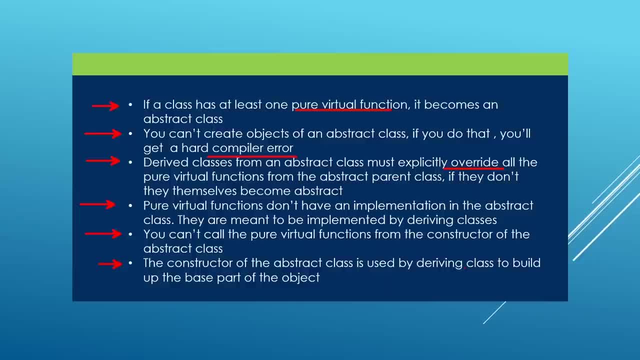 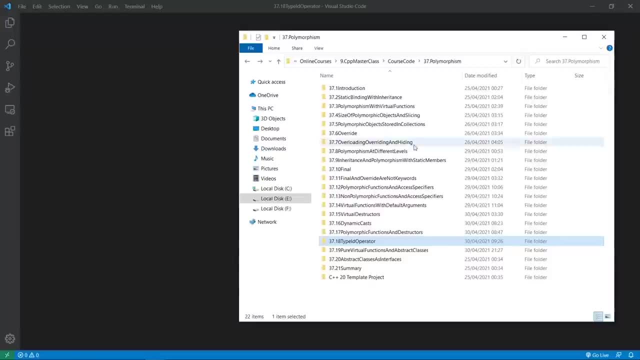 be used from the outside, because we can't really create an object of an abstract class. so now that you notice, we're going to head over to visual studio code and play with this a little more. here we are in our working folder. the current project is pure virtual functions and abstract. 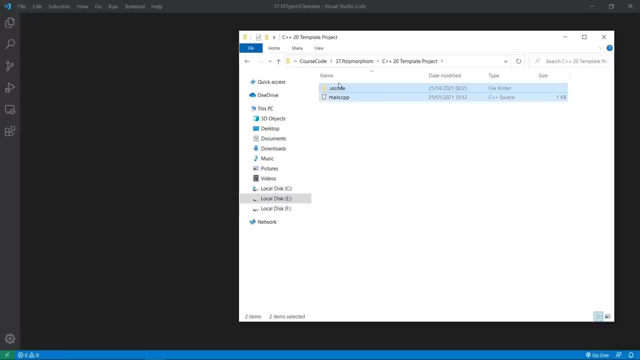 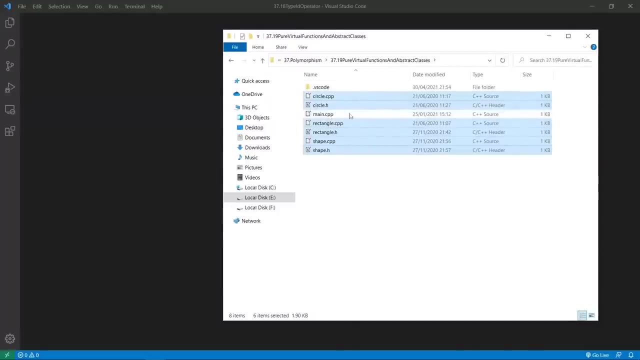 classes. we are going to grab our template files and put them in place and we're going to paste them in this project here and we are going to grab the files that make up our inheritance hierarchy. you are going to get these files from the resource section of the course. if you want, you can download. 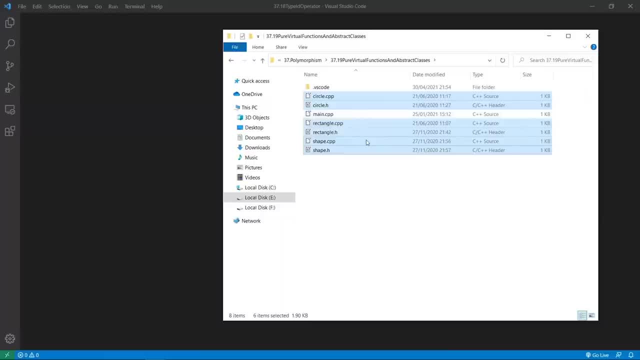 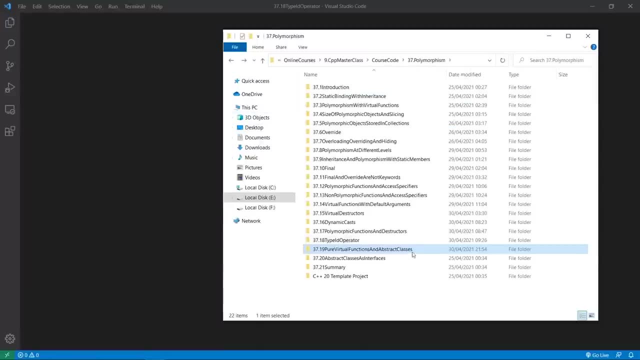 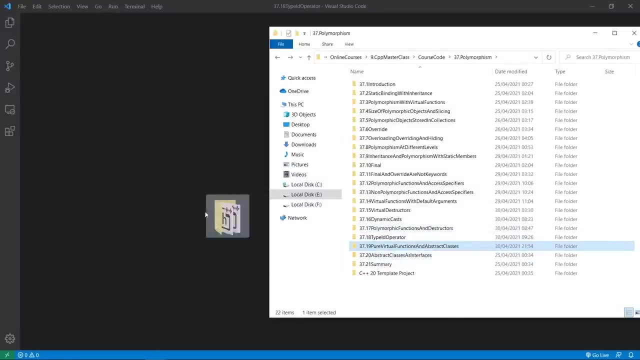 them and use them like i am using them here, or, even better, you can type the code and see how these things really work. that's the best way to learn. i do recommend that, but we want to save on time here, so i am just going to reuse these classes that i have lying on my drive. i am going to open 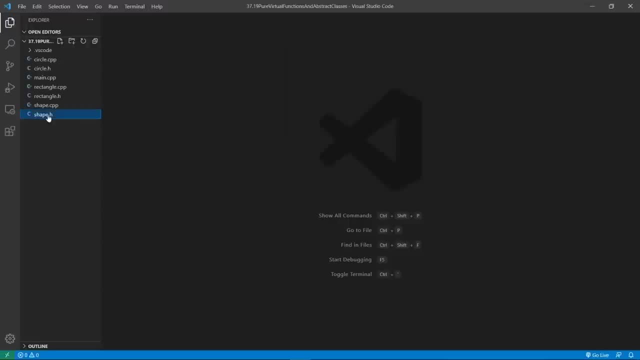 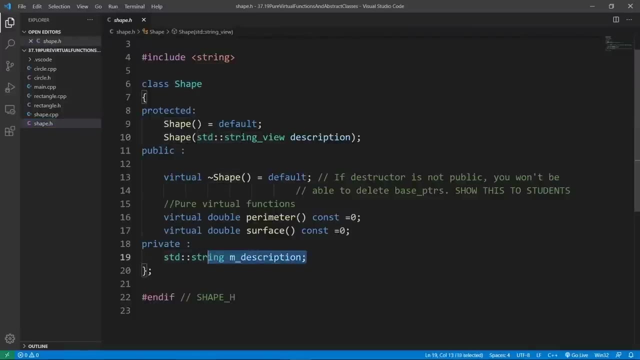 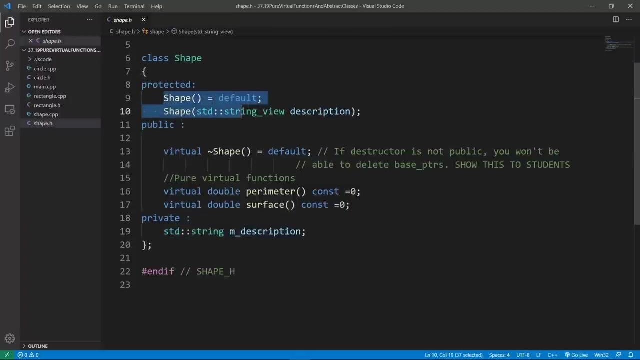 this and visual studio code. by dragging and dropping here, we have our shape class here. this is going to be our base class. you're going to see that we have our member variable, which is going to be the description for our shape. we have a bunch of constructors here, but the most important thing- 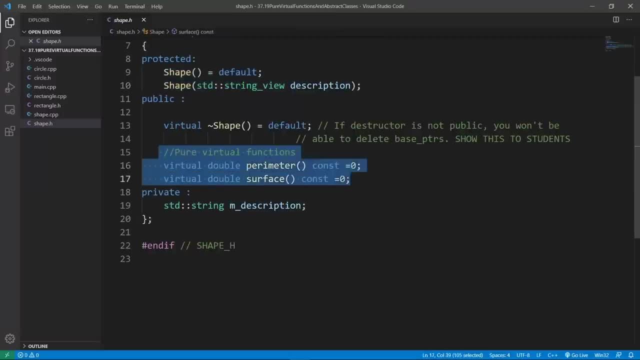 here is that we have a bunch of pure virtual functions here and if you go in the cpp file you're going to see that we don't have implementations then for the perimeter and surface. these are pure virtual functions and we have no business putting in an implementation in the base. 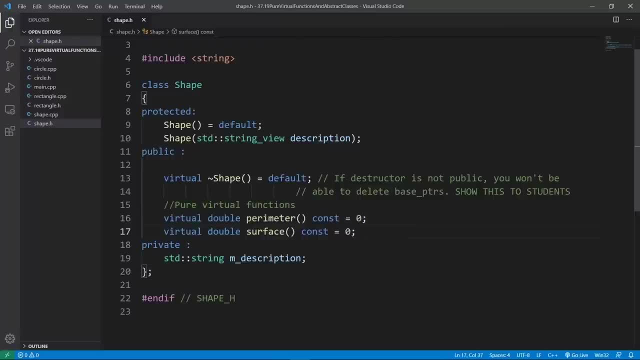 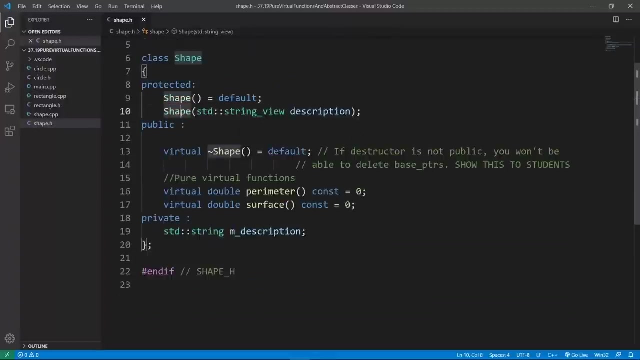 class. once we have these virtual functions in and mark them as pure virtual functions by prepending an equal zero here, this class here is going to become an abstract class and what that means is that we can't create objects of this class. it is meant really to be inherited from and downstream. 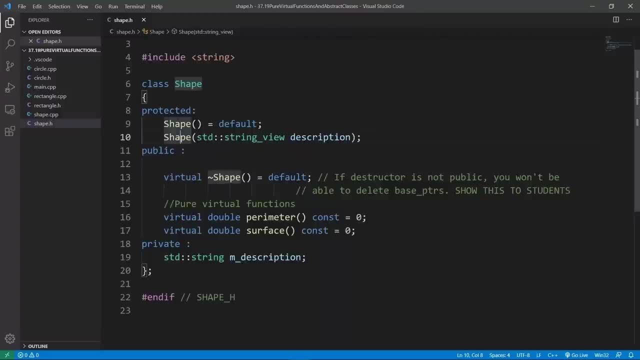 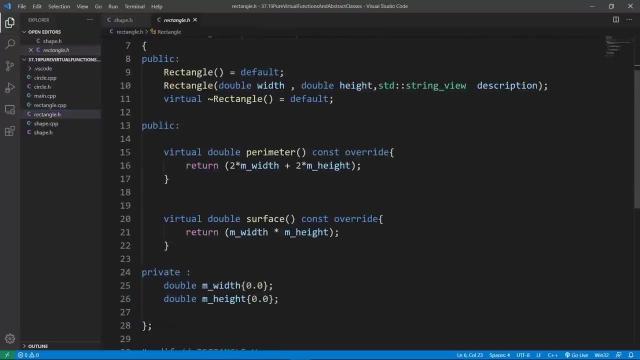 inheriting classes are going to be forced to override these methods here, otherwise they are themselves going to become abstract classes. we're going to have a chance to look at this here. we also have our rectangle class, which is going to be inheriting from shape. it is going to override our two methods. we're going to override 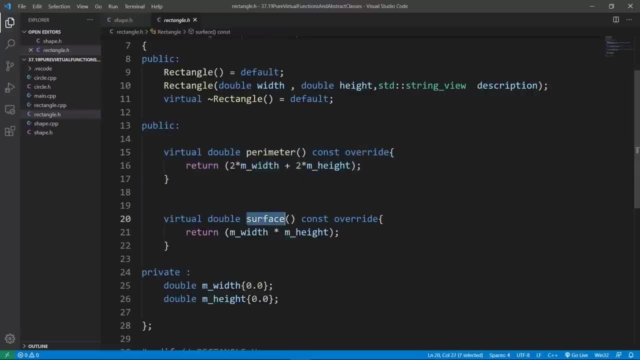 the perimeter function. we're going to override the surface function for rectangle. the perimeter is computed this way: we're going to multiply the width by two and the height by two and we're going to add this two things up. we're going to compute the surface by multiplying width and height and this is going. 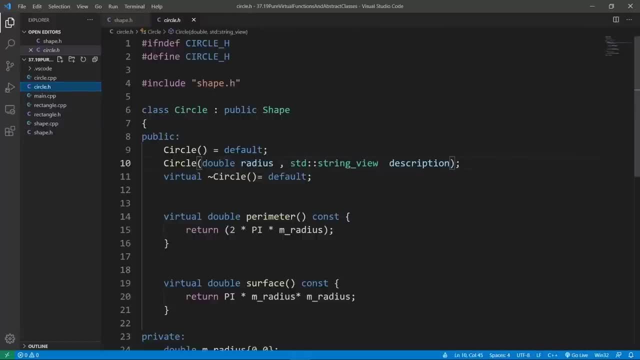 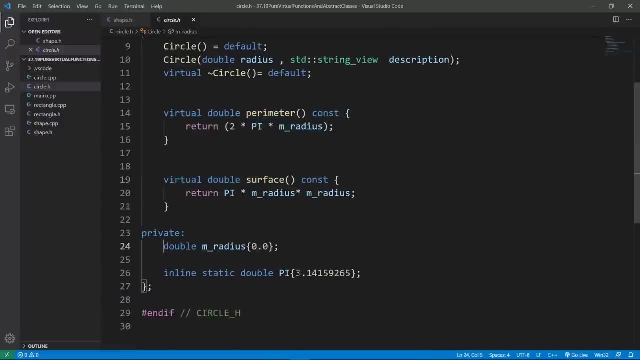 to give us the data we want. we can look at circle. it is going to also inherit from shape and it is going to override our methods here. if we want, we can even put in a radius and a variable to keep track of pi. we can do this, you can really do this, however you want. this is just going to allow us to. 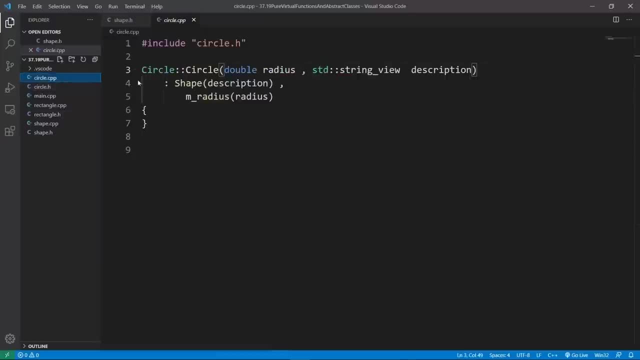 compute the surface relatively easily in this class. here let's look at the implementation. nothing special here. this is just going to allow us to compute the surface relatively easily in this class, where we would just give it a ctrl plus i in the JSON column and we're going to say that. 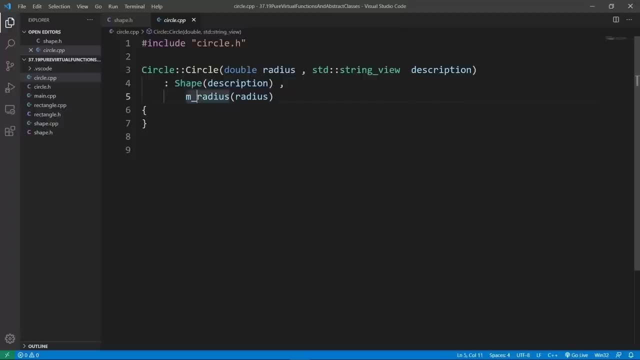 in the javascript class. we want to Romeo with our good parameters. so let's say we want the surface to be less than our belly width. this is going to be 47 degreesäus and we're going toalie our lineart from this lineart from our. 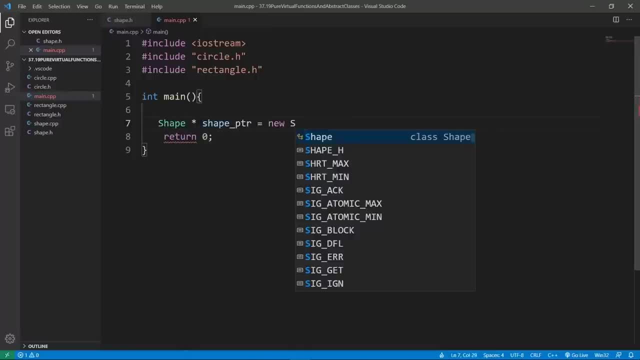 javascript class into theuez parcel command獍, the surface, and then we have cold electronics here, and this is not what we want. pointer- and this is going to be new shape- we can use a default constructor and if we do something like this, you're going to see that we're going to have a compiler error. here we have a squiggly line. 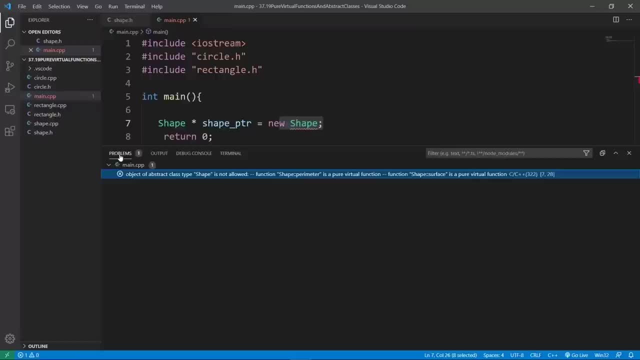 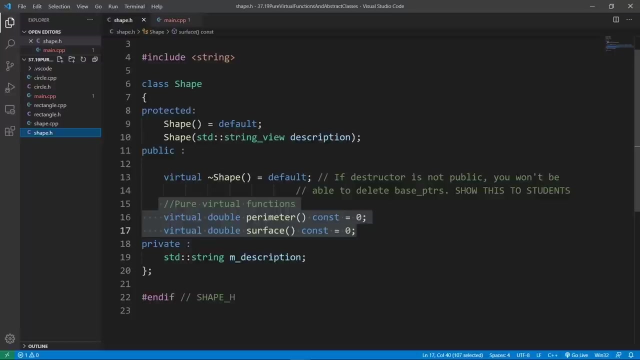 but if we bring up a terminal window and look at the problems tab, we're going to see that object of abstract class type shape is not allowed. so shape is an abstract class. now, and why is it an abstract class? because we have in at least one pure virtual function. here we actually have two. 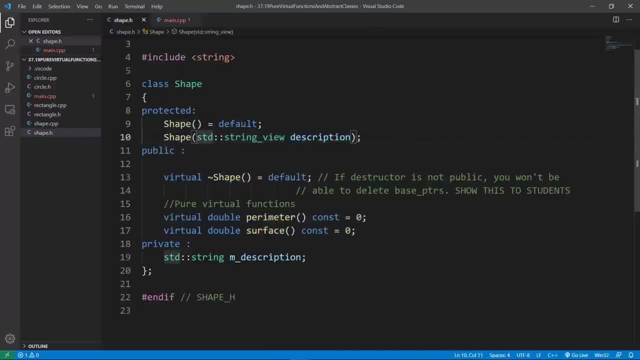 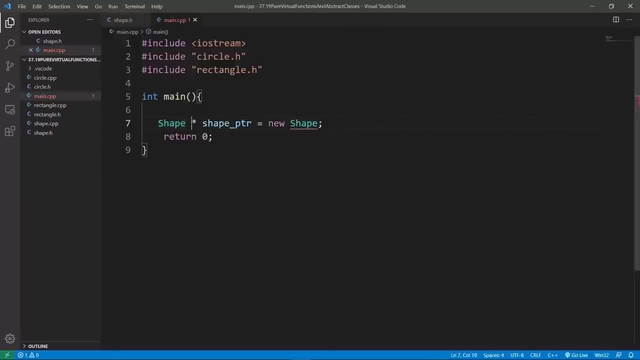 and this is going to make our shape class an abstract class. what that means is that we can't create objects of this class, and if we do that, we're going to get a compiler error. let's try and build this program. we're going to pass this through gcc, our favorite compiler. we are going to 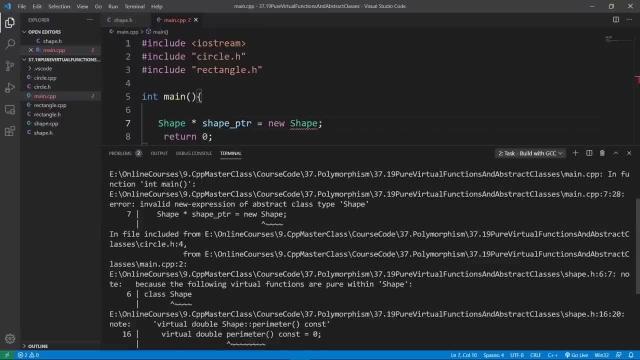 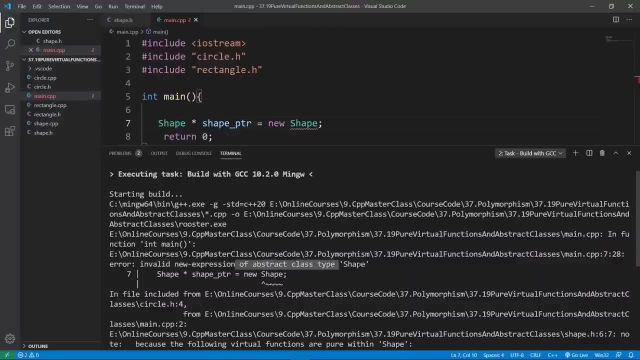 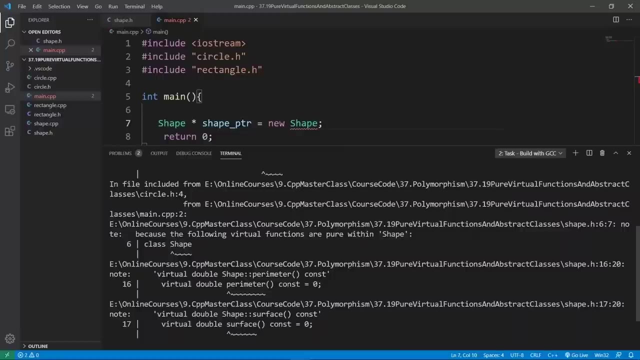 see that the build is going to fail. we're going to have a bunch of errors. if we go up and look at the error, we have invalid new expression of abstract class type shape, so we can't really create an object of this. let's go down and see what these errors are saying. note, because the following virtual functions are: 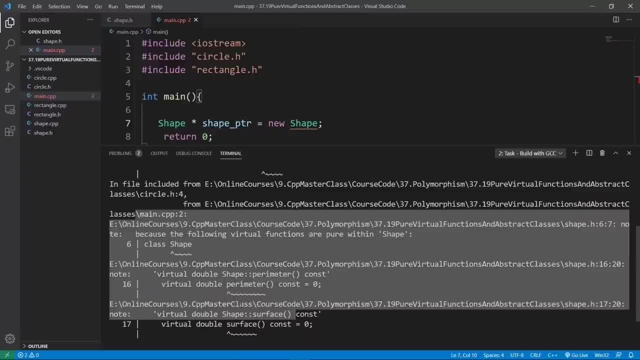 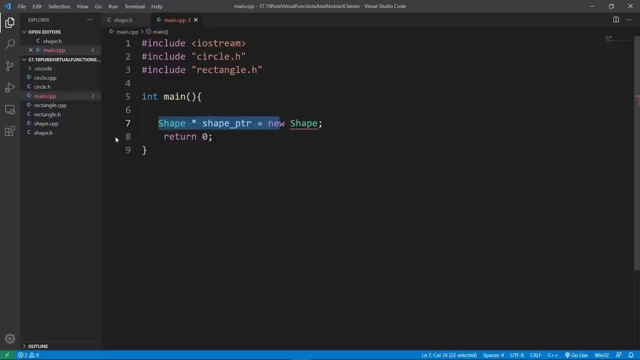 pure within shape and they are going to try and really be helpful in the errors that they give here. and all they are saying is that we can't create objects of this class because we have pure virtual functions inside. okay, now you know this. if a class is abstract, you can't create objects of that class, but you can still. 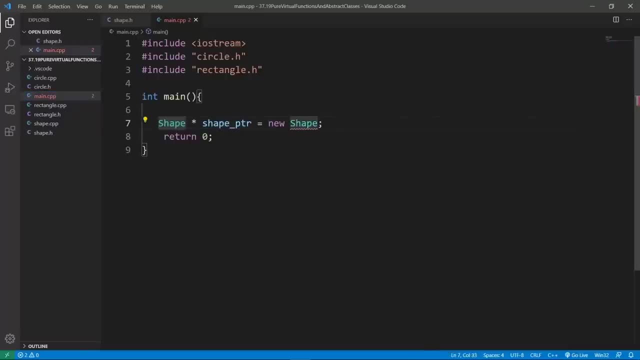 use a base pointer to manage derived objects of that class. so let's comment this out, because this is going to make our code not compile and we're going to say that this is going to give us a compiler error and we're going to try and use a base pointer to manage a rectangle object. we can. 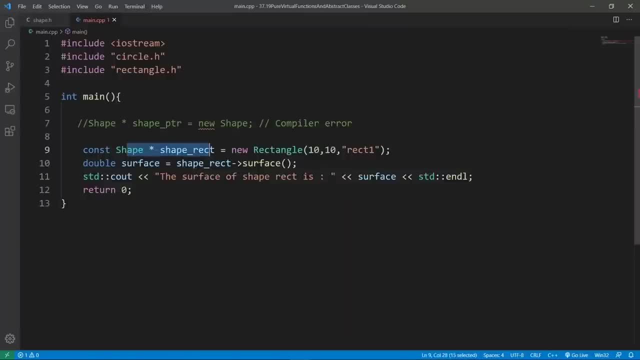 do this. so we're going to set up a shape pointer and it is going to be managing the memory of a rectangle object. we're going to go through the memory of a rectangle object and we're going to do the base pointer and call the surface method and this is going to call the implementation in. 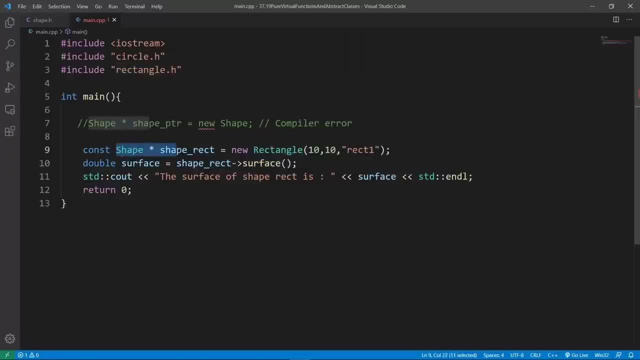 rectangle, because our base pointer is really managing a rectangle object. if you want, you can even use the type id operator to print the dynamic type of this shape rect pointer. you're going to see that it is managing a rectangle. you can actually do this because we learned about that in the last. 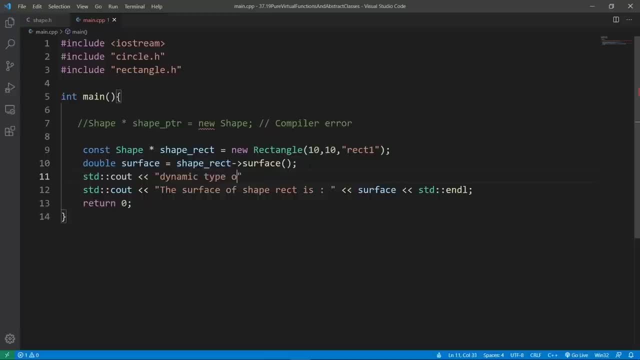 lecture. so let's practice that we're going to say dynamic type of shape rect and we're going to say type id and we're going to dereference the pointer. we're going to say shape rect and we're going to print the name of this and we're going 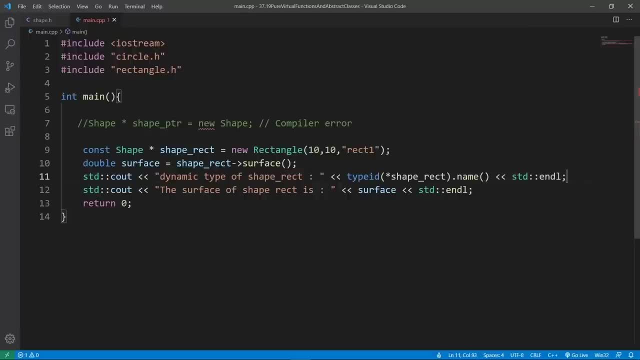 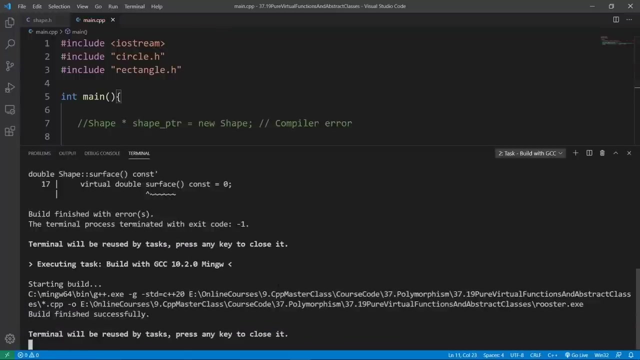 to see it print out on our powershell window and after this we are going to print the surface that we got from this call here and we're going to see what this gives us. let's try and build this program. we're going to pass it through gcc, our favorite compiler. the build is going to be good. 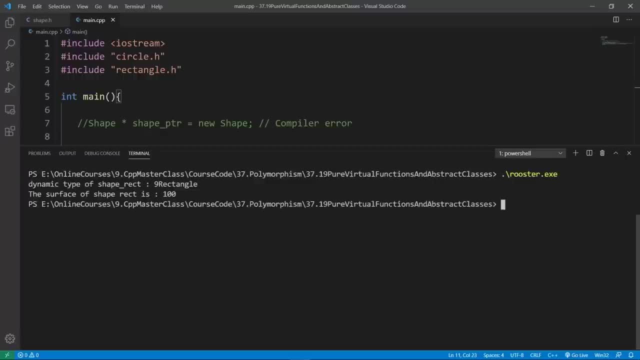 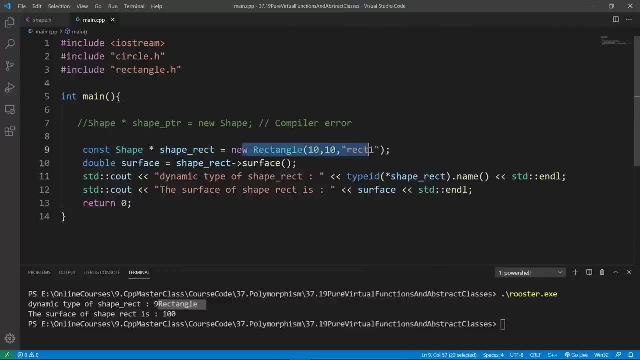 we're going to clear and run rooster, we're going to see that the dynamic type is rectangle. you can see that right here. so the base pointer is going to be the dynamic type and we're going to see that it's really managing a rectangle object. and this is what we have here. and if we call the surface, 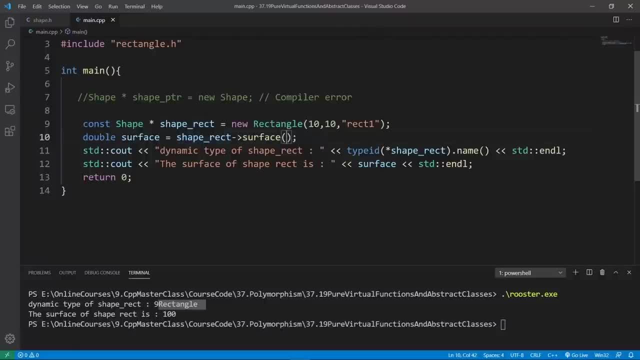 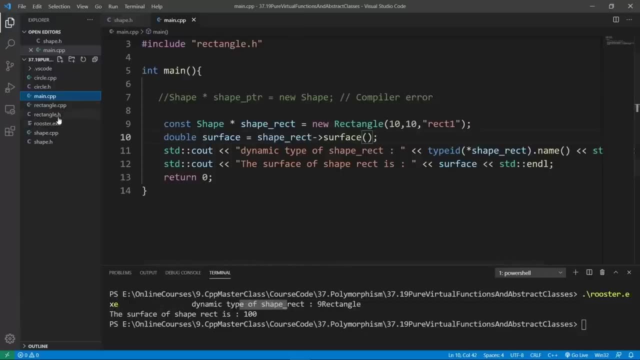 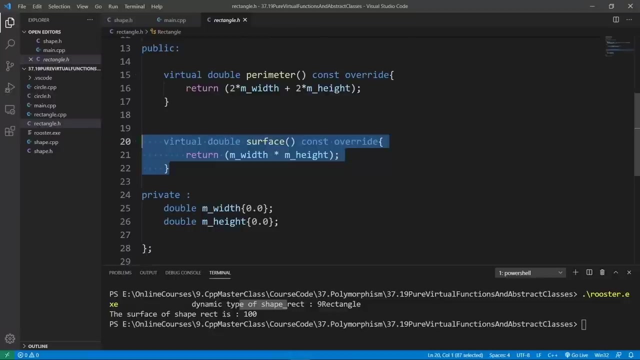 method. we will be calling the method on the dynamic type. so we will be calling this surface method on the rectangle class and we will be using the implementation we have here. so the surface function that is going to be called is what we have on line 20 in rectangle here and this is: 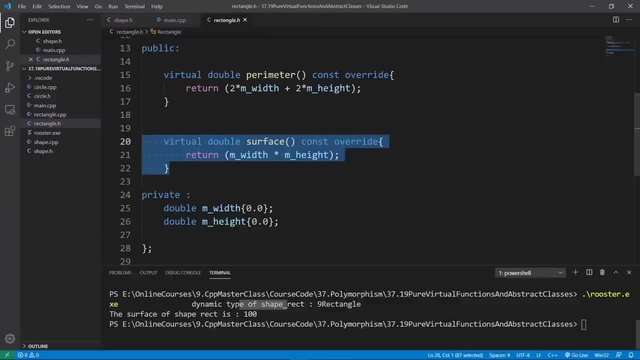 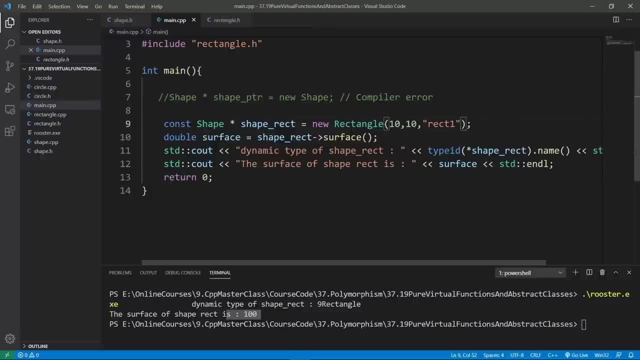 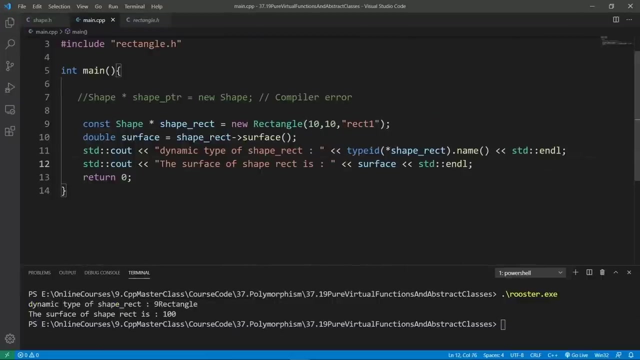 going to just be a multiplication of width and height, and we're going to get 100 here, because our width and height happen to be 10 and 10, so multiplying this is going to give us 100, as we see here. this is really cool. this is what we expect. we can even use our base pointer. 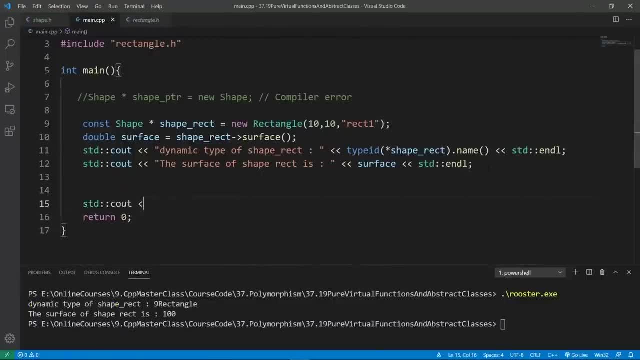 to manage a circle object. so let's do that. we're going to put in a separator to be able to follow this easily and our output. so let's say std and dl here and we're going to put in the code. so we're going to set up a base pointer which is really going to be managing a circle object here. 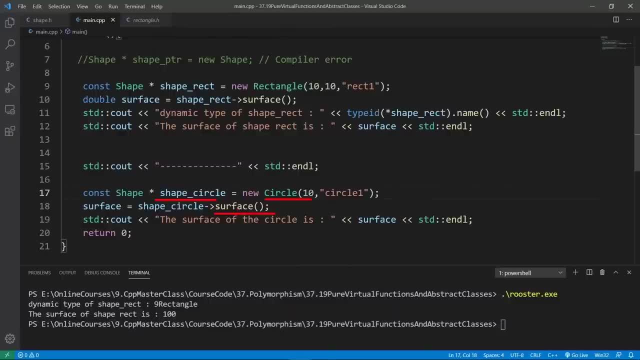 and we will call our surface method. this is going to call this method polymorphically, because surface is a virtual function, so we will get polymorphism here and we will call the surface method on the circle object, which is really our dynamic type. if we print this out, we're going to 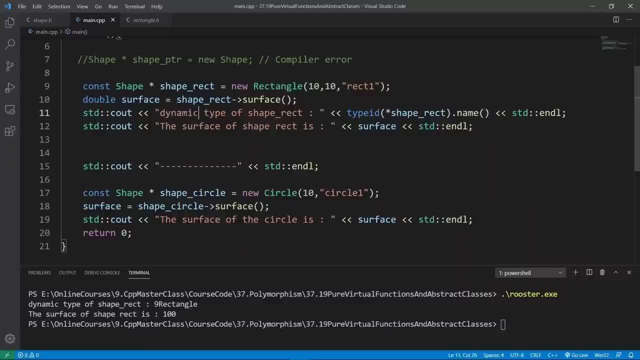 see the surface printed out. but if we want, we can even print the dynamic type of our base pointer here. so we're going to do the same thing we did for rectangle: we can use our type id to print the dynamic type of shape circle and we're going to say shape circle here and this: 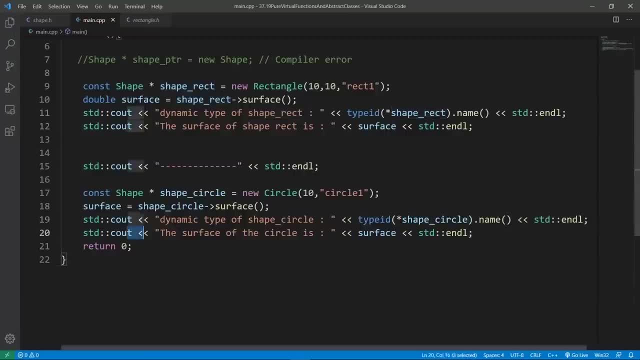 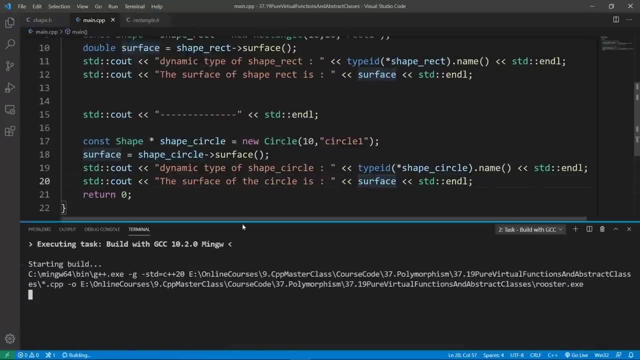 is going to do what we want. let's look at this. we're going to be printing the surface here. this is exactly what we want, so let's build and run. we're going to pass this through gcc. the build is going to go through, as you see here, if we clear and run rooster, we're going to see that the 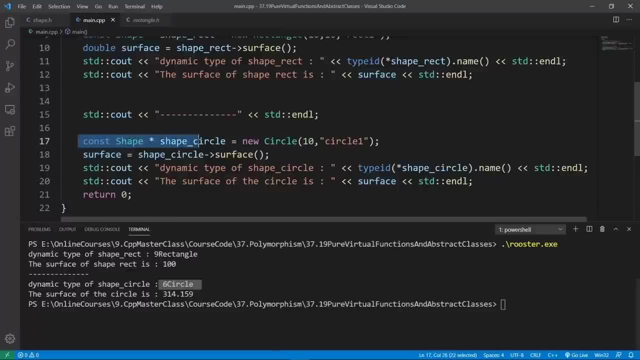 dynamic type is now a circle. so the base pointer or the shape pointer we have here is really managing a circle object polymorphically. so if we call a virtual function on this base pointer it is going to call the most specific implementation of the surface object we have. and that happens to be for 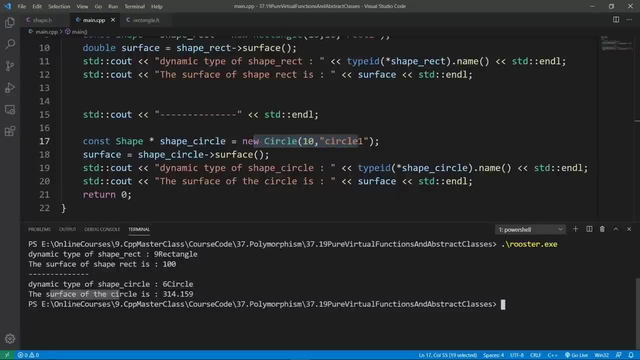 this circle object here. this is what i mean. if we compute the surface, we're going to see that it is going to be using the data we have here and we will get this number as our surface. if you plug this in, you're going to see that this is really right. so this is really all i had to share in this. 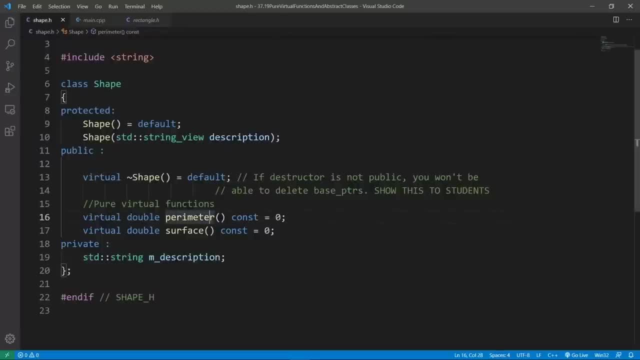 lecture. we can set up pure virtual functions in our base class and what that's going to do? it is going to make our class an abstract class. but we won't also be able to put in implementations for these methods anymore in the base class, because they are meant to be overwritten and implemented by 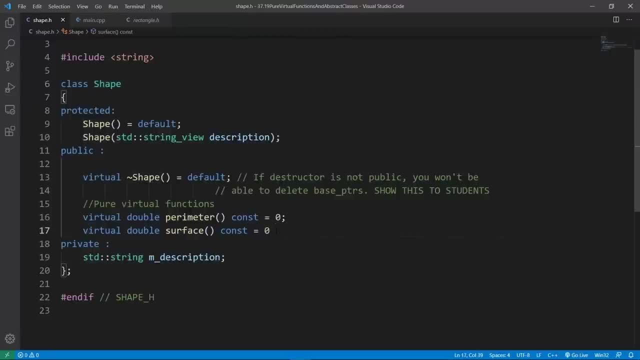 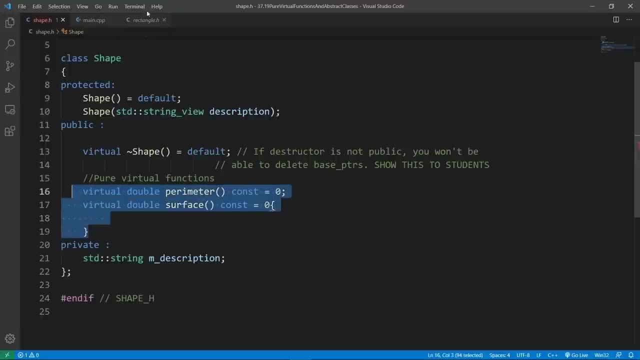 downstream inheriting classes. so if you go in here and try to put in an implementation, we will probably get a compiler error because this is not allowed. you see, we have a problem here. let's make sure let's import this here. if we try to build, we will get a weird compiler error. 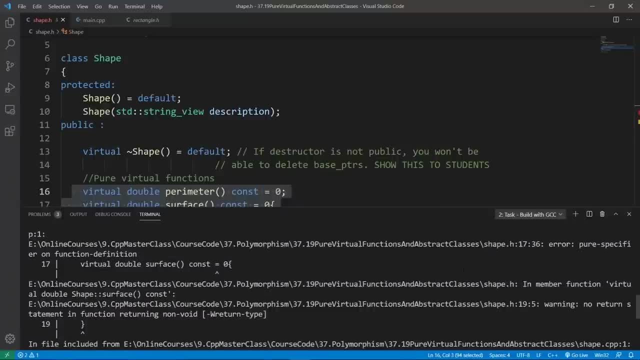 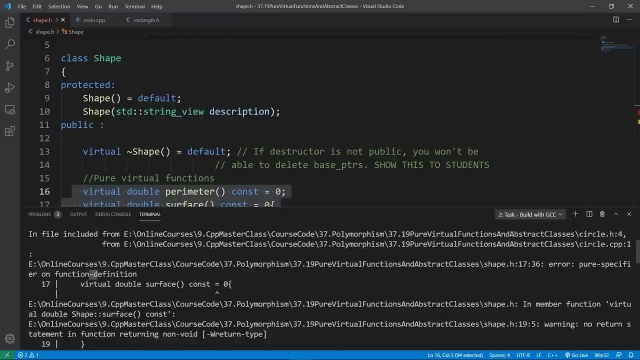 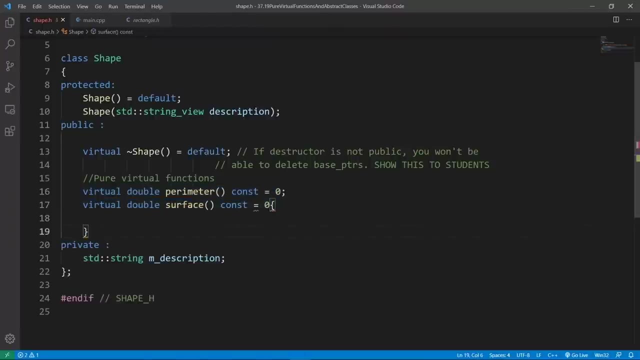 let's make sure we see the compiler error. so build finished with errors and we are going to see what's the problem here. let's go up and see pure specifier on function definition. so this is not allowed. so we are already conflicting ourselves here. we are marking this function as a pure virtual. 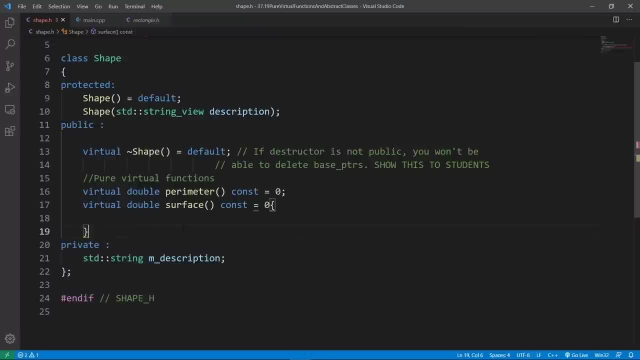 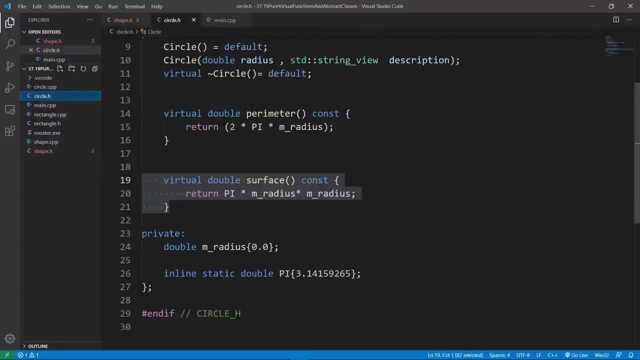 function and what that means. functions isn't meant to have a definition, but we are also putting in a definition here, so the compiler is going to be confused. this is not something we should be doing. another thing i want to point out before we wrap up this lecture is that downstream inheriting classes are forced. 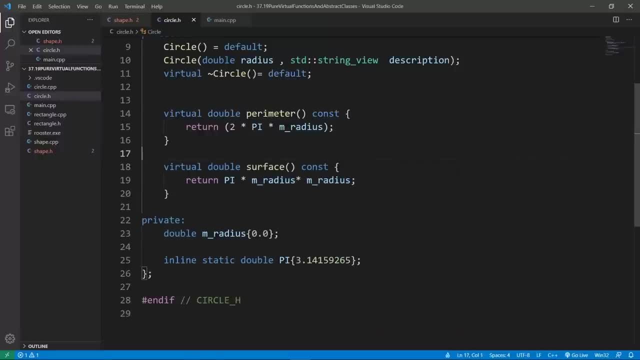 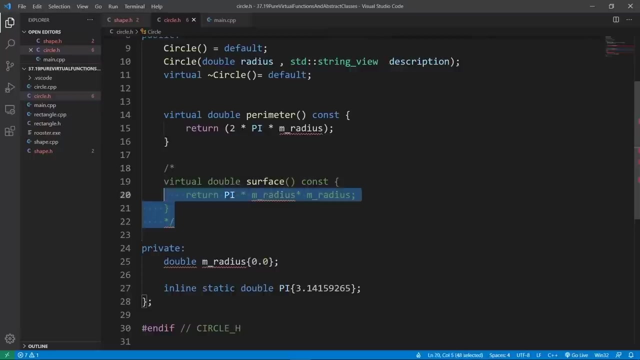 to override and implement all the pure virtual functions from the class that they inherit from. if they don't do that, they are themselves going to become abstract and we won't be able to create objects of them. so let's try and, for example, comment out the surface implementation here. 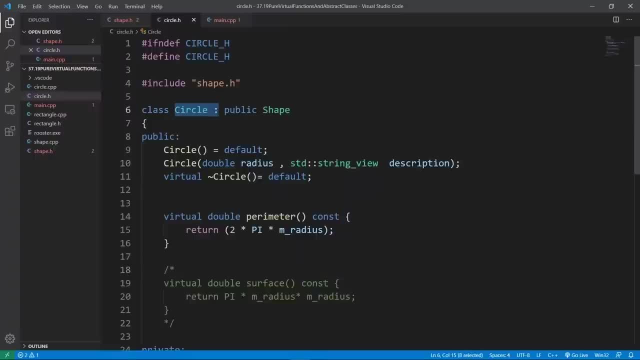 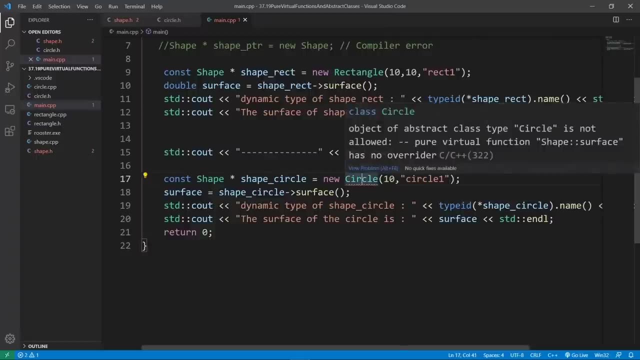 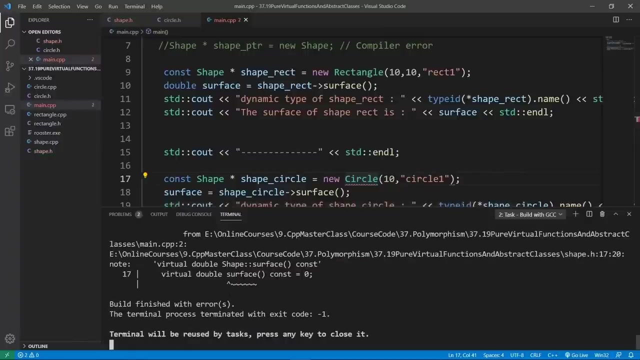 and that's going to make our circle class an abstract class. and if we try to create an object with circle, we will get a compiler error because now circle is an abstract class. let's try and build and show you the compiler error, and this can really be confusing if you are a beginner on this. 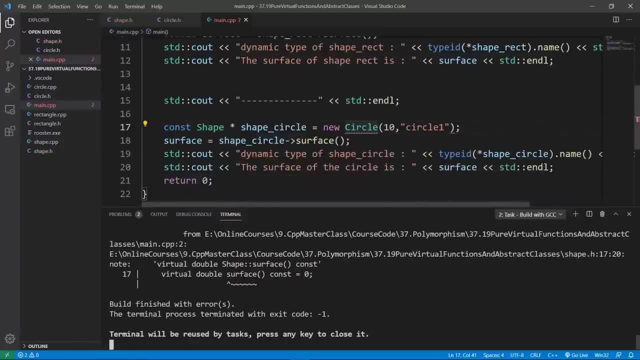 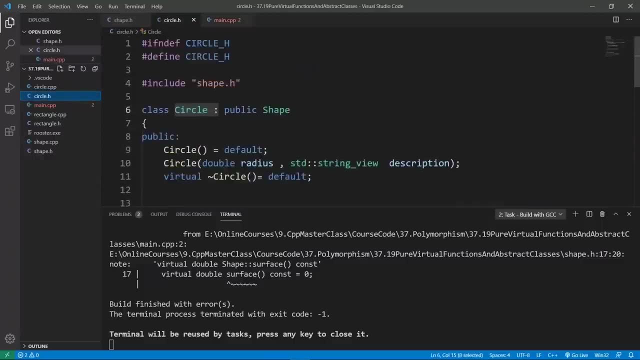 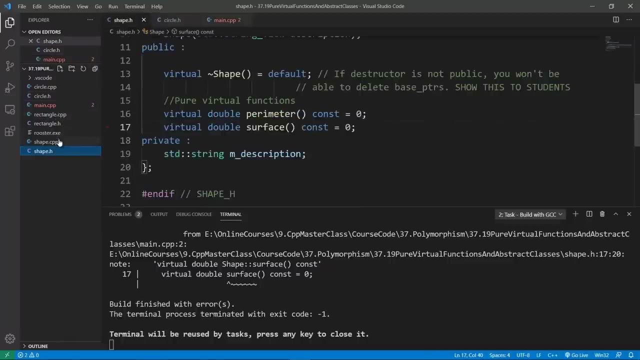 you will be wondering why you can't create objects of your class, even if you didn't really explain the structure of your class. so let's try and comment out the surface implementation here. the reason is we are inheriting from an abstract class that has two pure virtual functions, but we 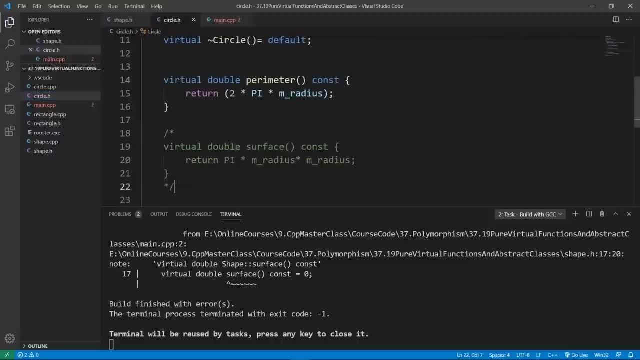 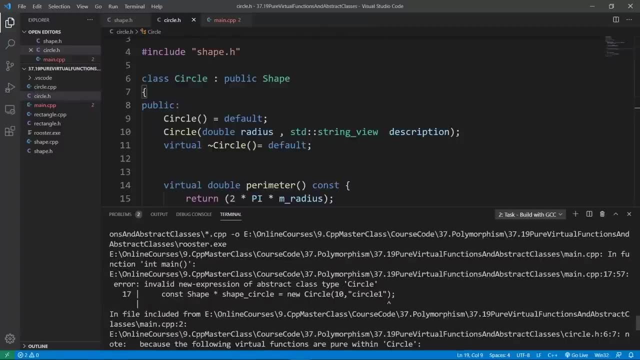 are only overriding one pure virtual function. we need to override all of them, otherwise our class is also going to be an abstract class. let's look at the compiler error we are getting here. let's go up and see if we can find it. we are going to say in function in main: invalid new expression of. 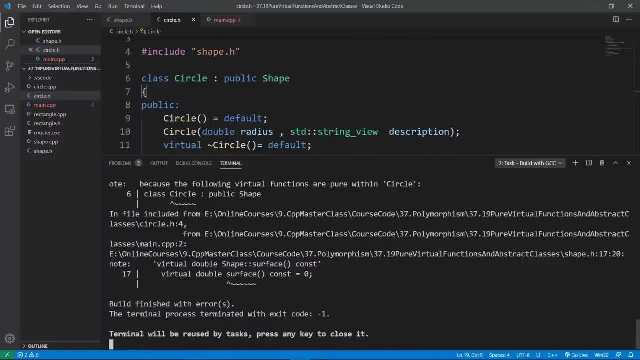 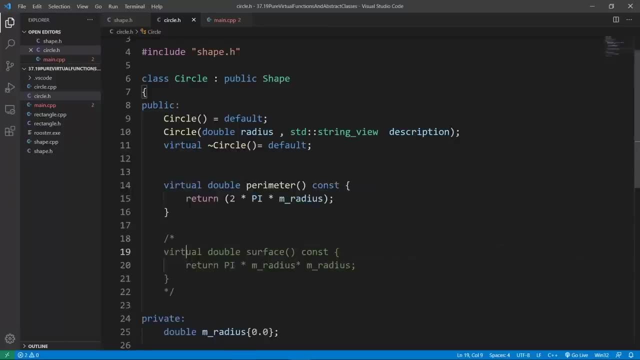 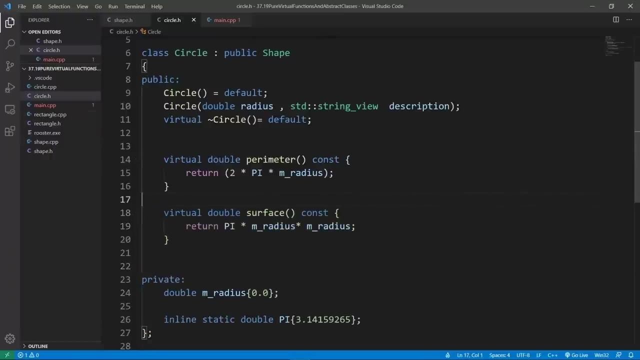 abstract class type circle. we are trying to create an object from an abstract class. this is the error we have here and you should really know this. so let's go back and make sure we are overriding all these things, because we need to do that to be able to create objects of a circle. and now this is going. 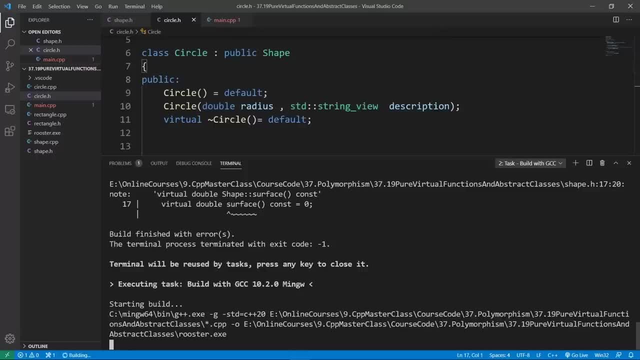 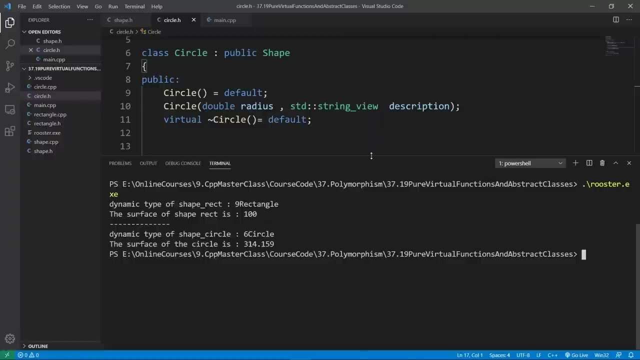 to work exactly as it should. let's build and make sure of that. the build is going to be good. we are fine. this is working exactly as we want. this is really all i wanted to show you today, so let's go through the scenes. Lindsay, some of you probably who, like um, actually attended the lecture, right? 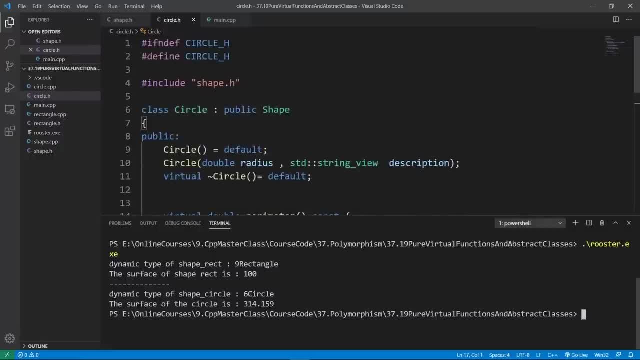 now let's appreciate what we picked out of this video. if you enjoyed it and consideryani, thank you so much for staying until the end of the video. and before we end today, i want to say: all of you really feel the hug. you want to cherish this友虞. every day we forget to. 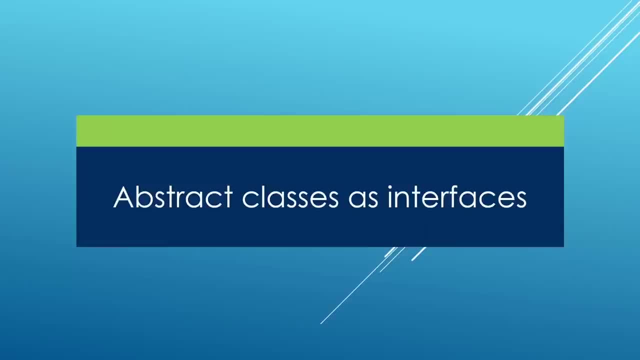 that let's uh leave the conversation that everyone should know. the exam was so easy, so i hope that was lucas's demo and i hope you liked the video, so remember to subscribe. hit the bell if you want to receive more and all the latest updates when i upload a new video and also 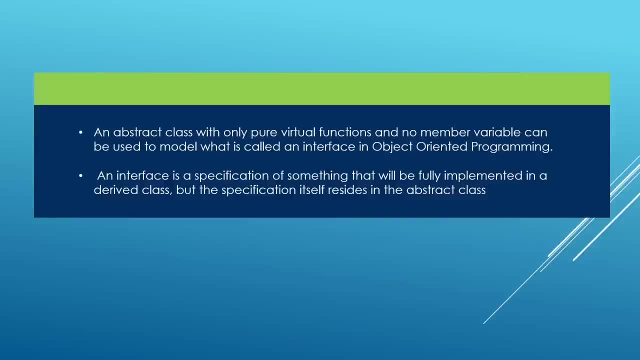 An interface can be thought of as an abstract class with only pure virtual functions and no member variable. So if you have a setup like that, you can call that thing an interface. Let's look at a simple example here. Here we have a simple class called stream insertable. 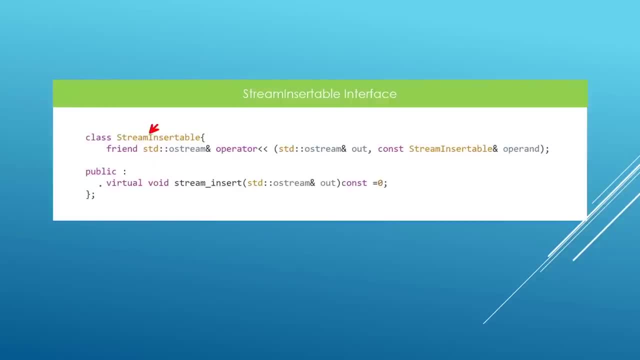 You see that it doesn't have any member variable. It only has a pure virtual function here and a helper function that we could set up to help us do a few things. The only specification to make this an interface is to have in only pure virtual functions and no member variables. 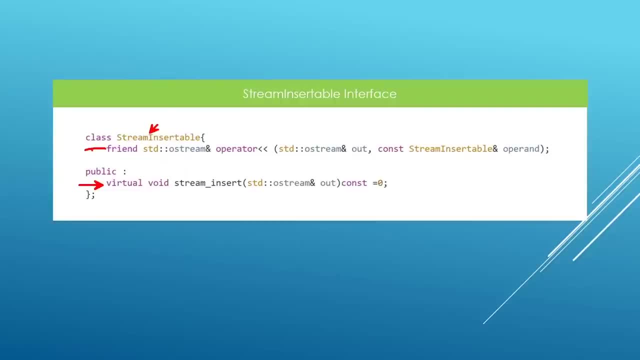 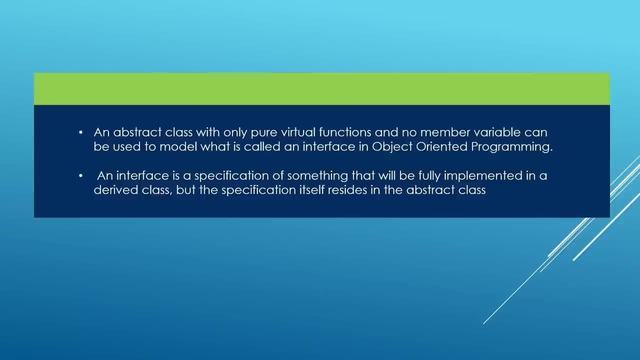 If you have in a member variable, this is going to stop becoming an interface in C++. OK, so you can think of an interface as an abstract class with at least one pure virtual function and no member variable. That's going to make it an interface. 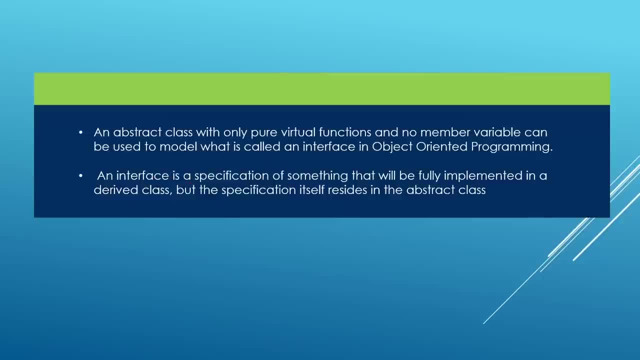 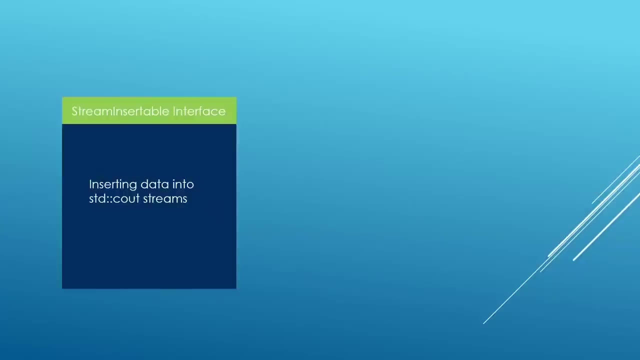 Down here you see that an interface can be thought of as a specification of something That will be fully implemented in a derived class, but the specification itself is going to reside in the abstract class. Another way to think about an interface is to treat an interface as a thing you can attach to your types to give them superpowers. 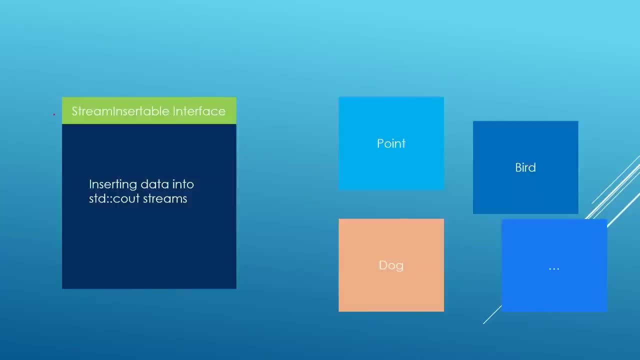 For example, this stream insertable interface has a single job and that's going to allow our types to insert data into output streams like HTTP. This is the only thing this interface is going to add to our types. So we can take this interface and attach that to a point class, for example, and we will automatically be able to print point objects to the output stream. 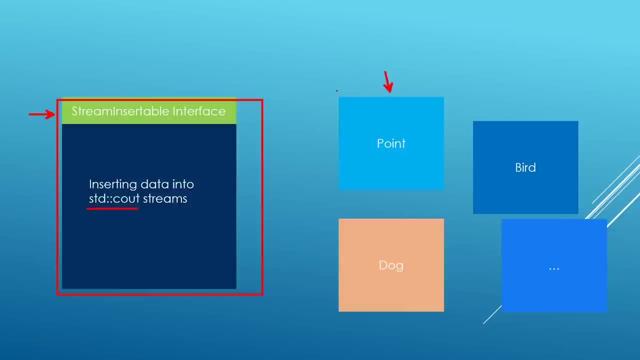 And we want to need to overload the stream output operator in the point class, We can do the same thing to our bird class, We can do the same thing to our dog class and we'll be able to print these things without having to overload the stream output operator. 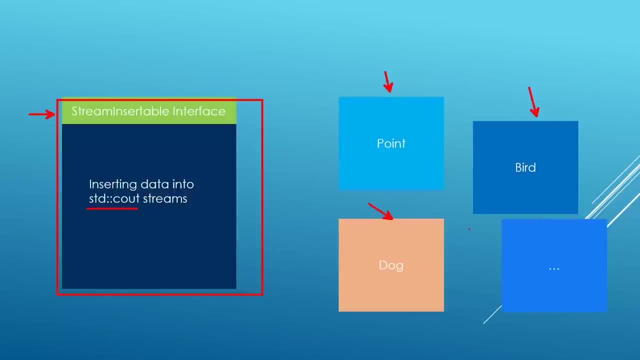 Hopefully you can see how powerful this is if we manage to set up this kind of relationship between our type and our interfaces. So again, an interface is something you can attach to your types to give them powers or features that they originally didn't have. 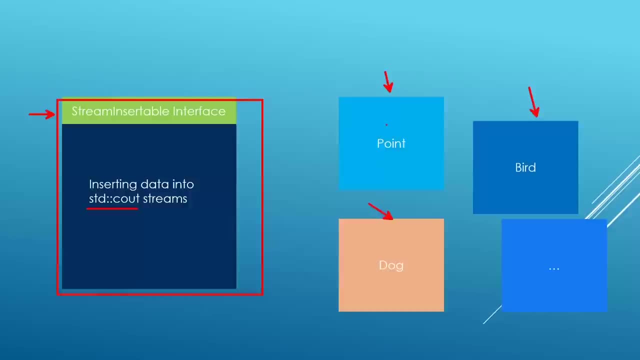 And that's going to save you from having to implement these features separately in each class for your time. So this is a huge time saver. Now you must be asking: how do I take my interface and attach it to my time? Well, the way C++ does this, you have to inherit from the interface, from your type, to attach the interface to your time. 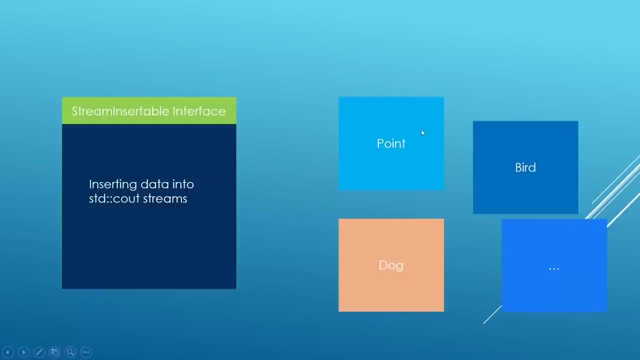 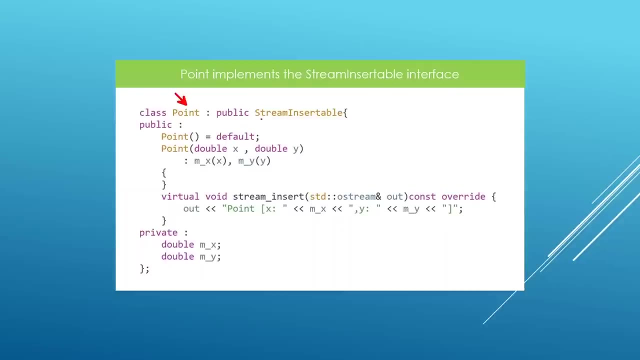 So, for example, if we wanted to attach this interface to our point class, what we would do is something like this: We would set up our point class and inherit from our interface, which is stream insertable. The moment we do this, our point is going to be able to print things to the console through the stream output operator. 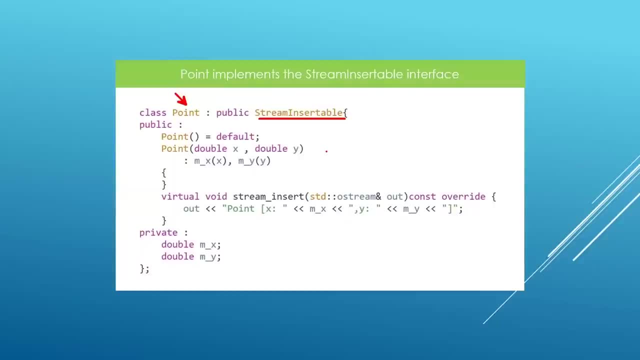 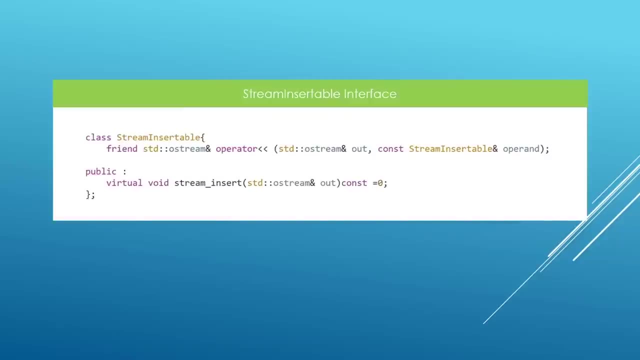 But hopefully you can see how powerful this is. We're going to see that something is missing. How does our point class know how to print stuff? If we go up and look at our stream insertable interface, we're going to see that it is declaring a stream output operator. 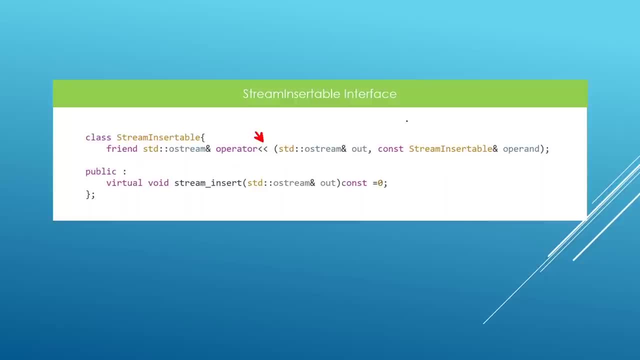 It is this thing that is used to print data to the output stream. You see, this is a regular output stream operator. We will be printing to std oStream and the object is named out here and we will be printing whatever operand that is passed as a second string. 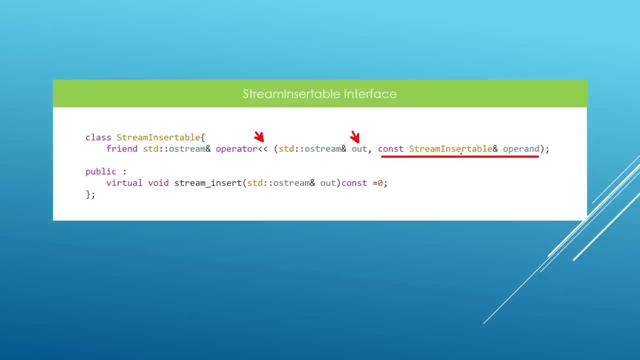 We will be printing to std oStream and the object is named out here and we will be printing whatever operand that is passed as a second string. We will be printing whatever operand that is passed as a second string, But the catch is we will need to set up a virtual function that will need to be implemented by whoever inherits from our interface here. 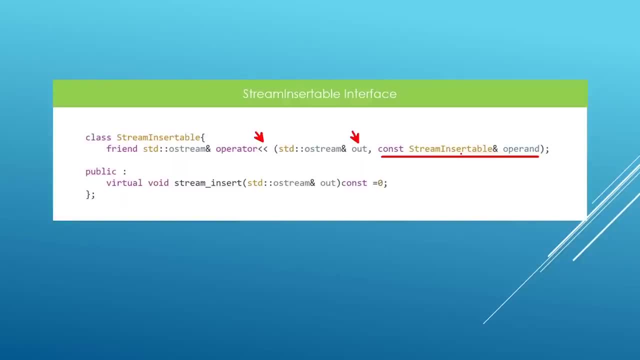 And this is going to be super powerful. We are going to take over the job to print to the output stream, but we will let inheriting downstream classes to specify what we print And they are going to specify that in this virtual method. Let's look at our point class again. 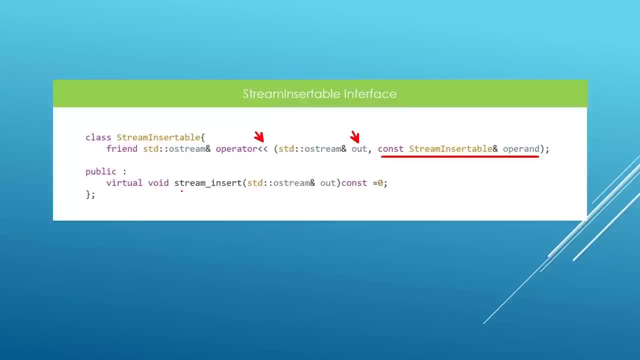 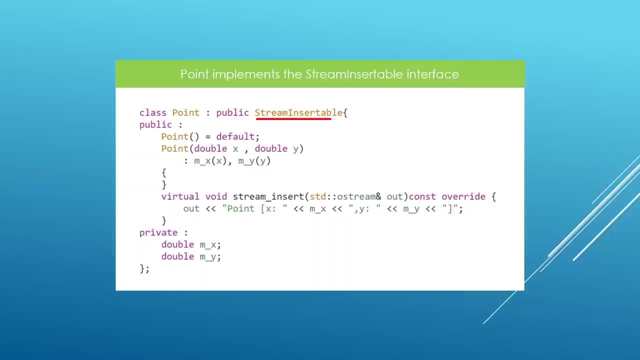 And really put the puzzles together here and understand how this works. Okay, this is our point class and it is going to be inheriting from our interface and it is going to implement our virtual function here. We are going to set it up here and we are going to mark it as an override, because it is overriding a method that comes from our stream. insertable interface here. 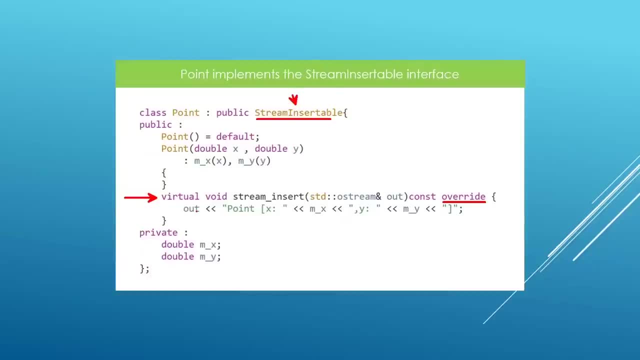 And it is going to specify which data we print to the output stream and how the data is going to be printed out. You can specify these things here. We are going to format the data in a point and we are going to be using these square brackets to put mx and my here. 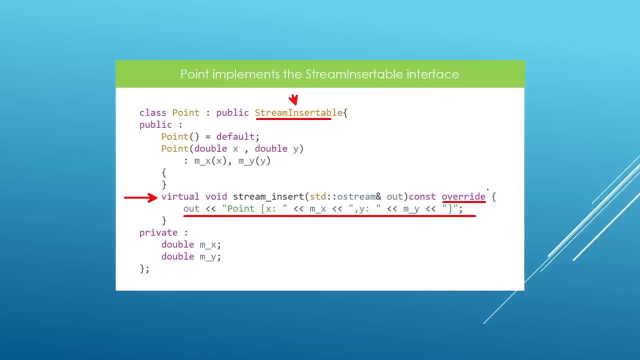 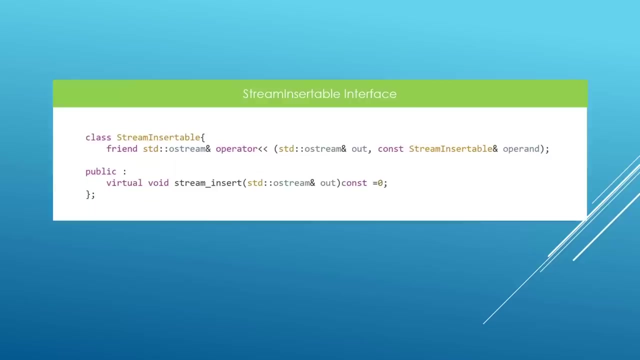 And notice that this is an override. So the inheriting class has all the information we need to put in our output stream operator, and we will do that through our stream insert override here. Now let's go back to our stream insertable interface to see how our output stream operator actually works. 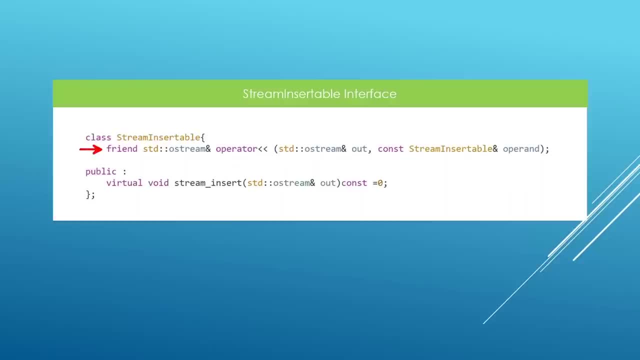 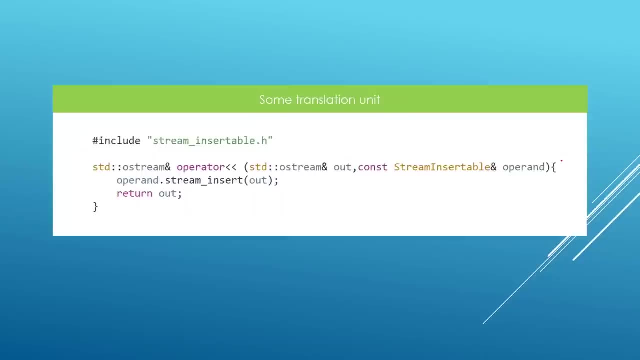 What we have here is what would be a header, and this is going to just put in a declaration for this, but we can even look at its implementation. The implementation for our output stream operator may look something like this: We are going to pass in the first operand and the second operand here, but notice what we are doing here. 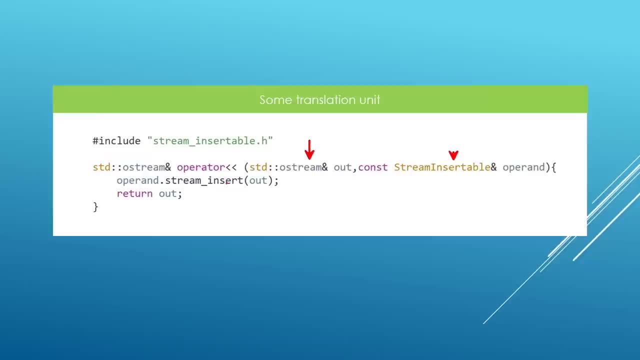 We are going to call the stream insert virtual function on our operand here And this is going to call the most specific implementation We can find for the stream insert. If we are trying to print a circle, for example, this is going to call the stream insert override on our circle object. 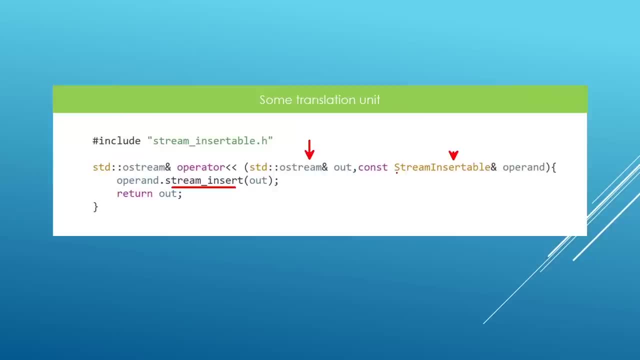 If we are trying to print a point, this is going to call this method on our point object and this is going to use polymorphism because our second operand here is passed by reference. Hopefully you can see how this is super powerful. I know this is convoluted because we are jumping around trying to explain this, but I couldn't really explain it. 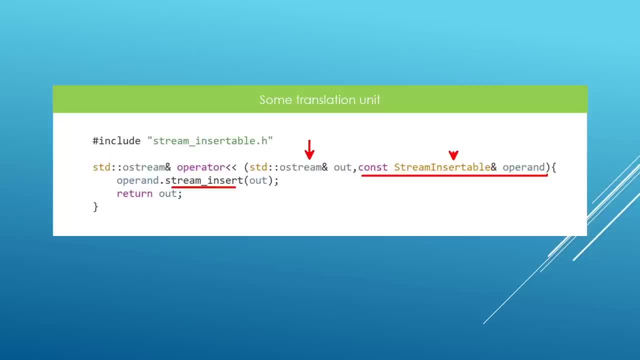 We have to try this in code to really see the power of this. but this is really the power of interfaces. We can design our features and wrap them in an interface and we can really attach that interface to any type we have in our C++ program. 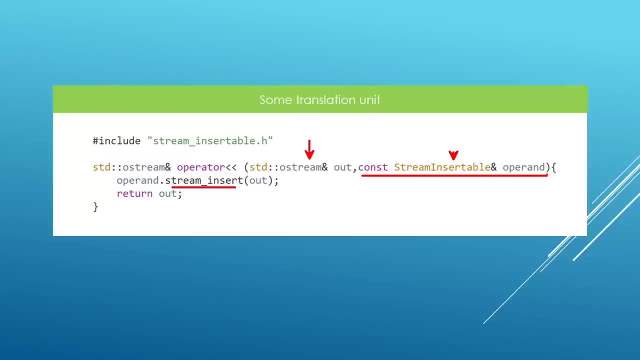 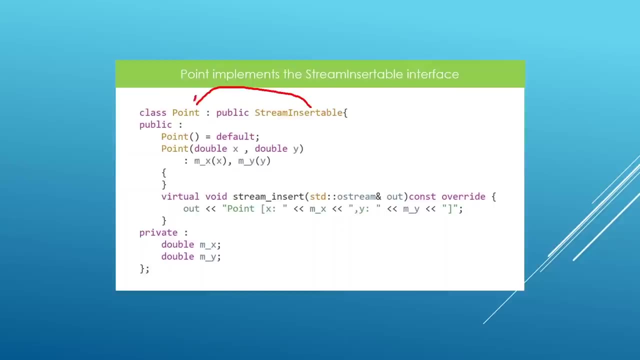 And that type is going to automatically inherit the features that we have set up in our interface. For example, now that we have attached this interface to our point here, we can print this If we print our points on the output stream, and this is going to work automatically. 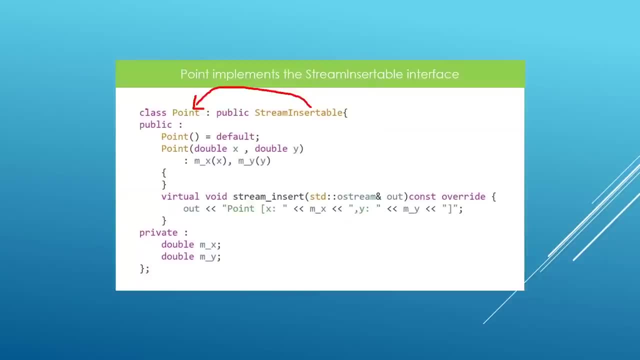 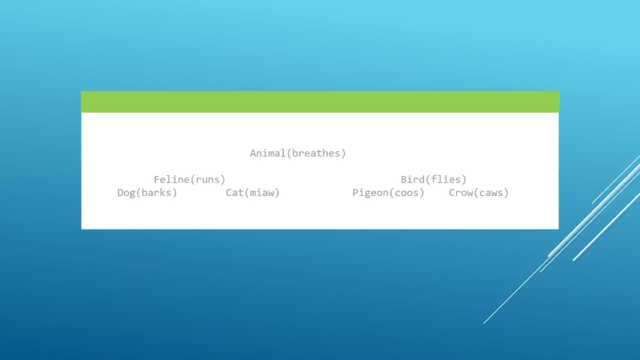 you see that we don't need to set up an output stream operator on our class altogether. We can even go further and attach this interface to a full inheritance hierarchy, For example, if we have our base class to be animal and we inherit from this class to create all kinds of crazy classes. 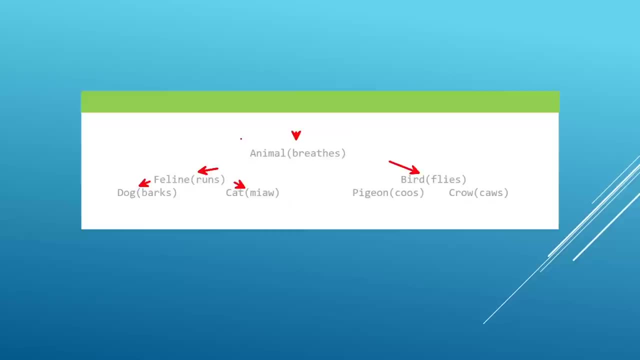 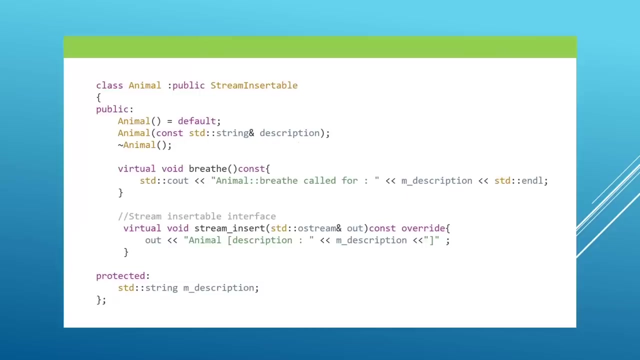 we can go on and attach our interface to the base class here. This is going to make all our classes in our inheritance hierarchy have the features that the interface has brought to the base class. So, for example, we can attach our interface to the animal class by inheriting from stream insertable here. 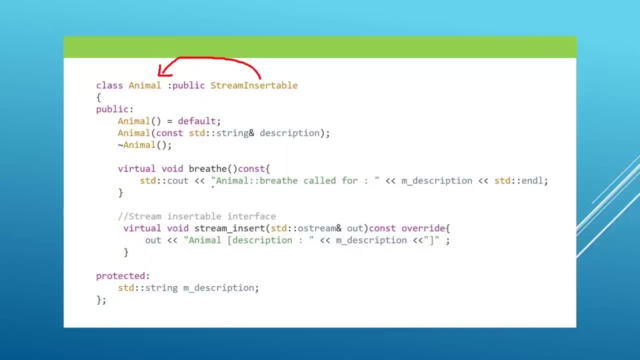 And this is going to give our animal the powers to be printed out to output streams, And this is going to be powered by the virtual function that we are overriding here. So, basically, we are going to specify which data to print in our animal class and how the data is going to be printed out here. 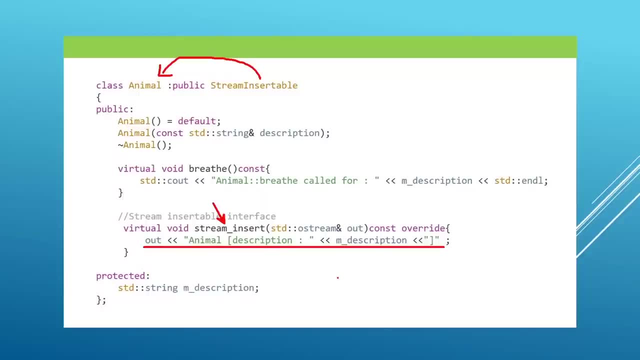 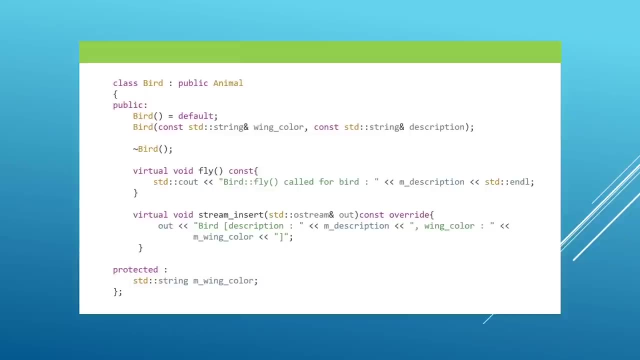 And we can do that in this override, And this is super powerful. Once we do this, we're going to go to each class in our inheritance hierarchy and implement the stream insert override, Because if we don't do that, this class is also going to become an abstract class, because it is inheriting from a class that has a pure virtual function. 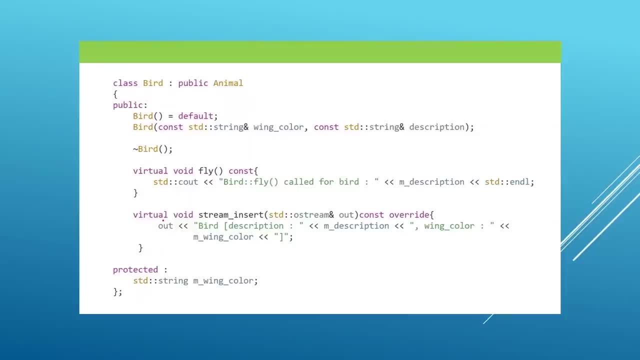 Remember, if you inherit from a class that has a pure virtual function, you will be forced to implement all the pure virtual functions that come from your parent class. If you don't do that, you are going to become an abstract class yourself, And we don't really want that. 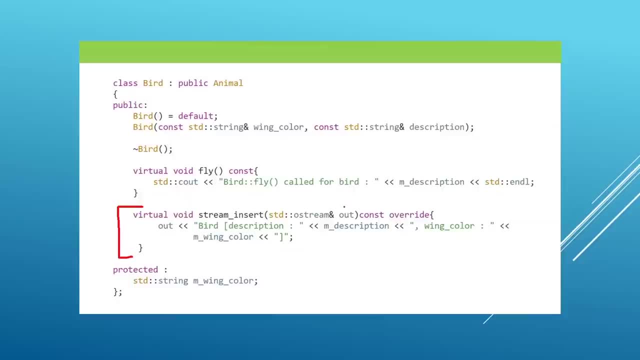 That's why we are overriding the stream insert override here And with this we are going to specify which information to print from our object here. In here we are going to put out the description and the wing color, And this is the format we want. 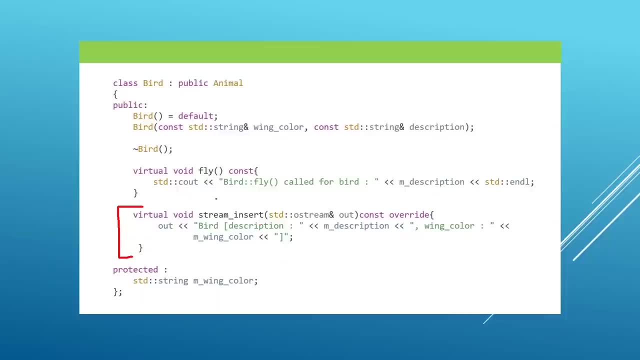 We specify here, And this method is going to be called by our output stream operator, which is coming from our stream insertable interface. Hopefully you can see how this is super powerful. Okay, now that you know this, we're going to head over to Visual Studio Code and play with this a little more. 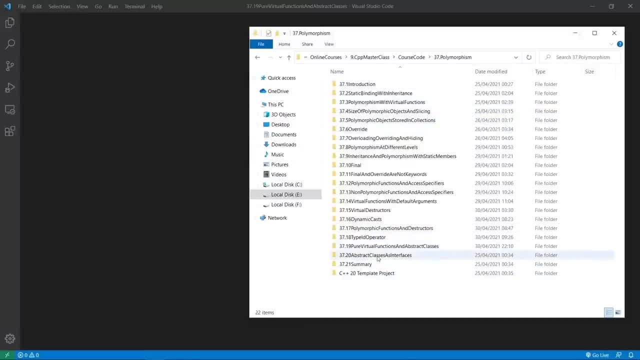 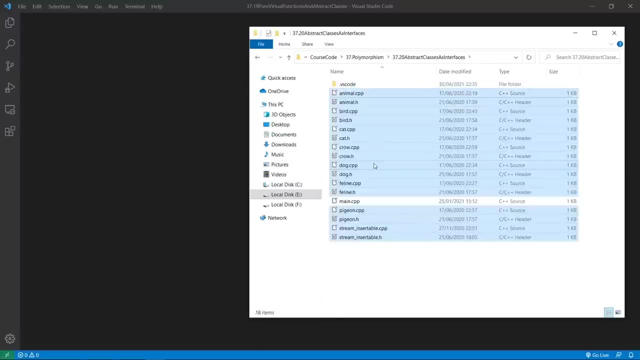 Here we are in our working folder. The current project is abstract classes as interfaces. We're going to grab our template files and put the data in place And I'm going to copy this and put that in here We are going to put in the files we're going to be using in our inheritance hierarchy. 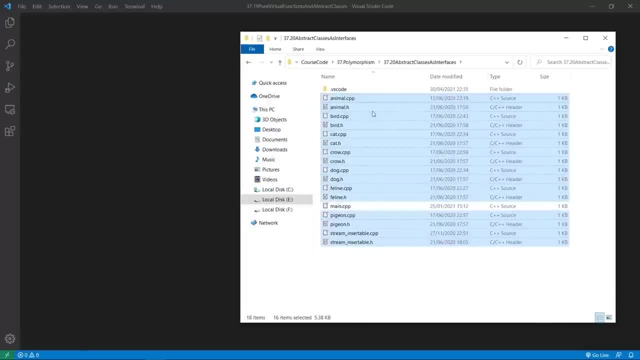 You see, we have our animal hierarchy here. You can grab these files from the resource section of this lecture and you can reuse them like we are using here, Or, if you want, you can even type this, But I don't really recommend this because this is too much typing. 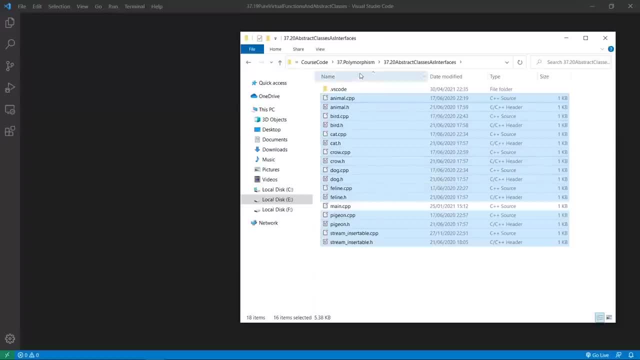 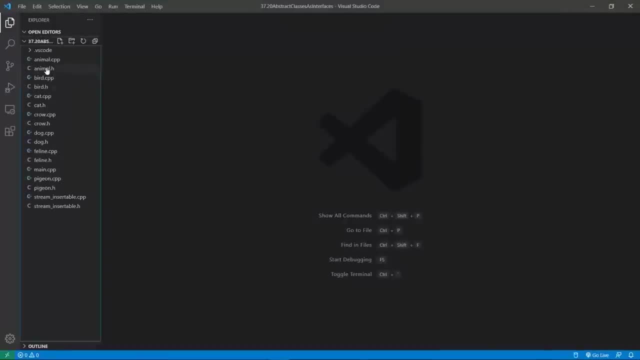 We just want to learn about interfaces here, And that's what you should focus on. So we're going to open this up in Visual Studio Code And this is going to give us all the files we need. We're going to look at the top class. 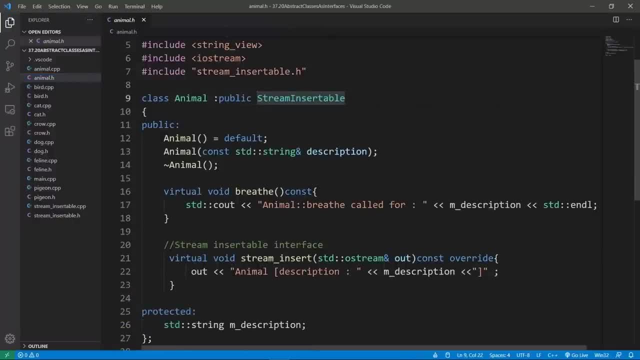 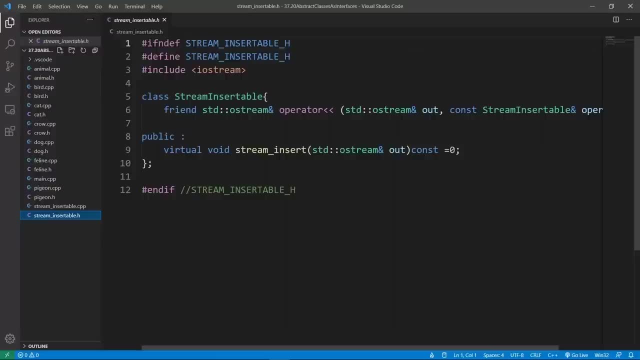 And we will see that it is inheriting from our stream insertable interface. So let's look at our stream insertable interface, because this is the focus of this lecture here. So it is a regular class, as you see, here It is class stream insertable. 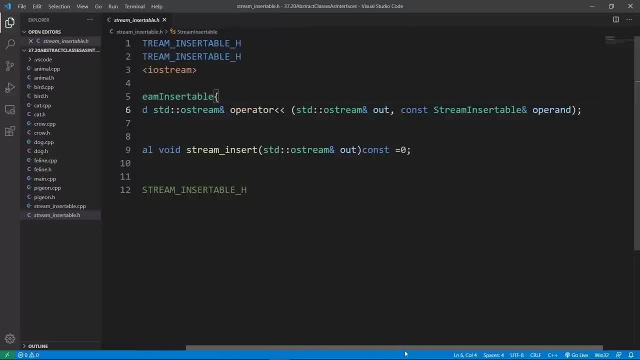 We're going to set up an output stream operator And it is really like any other output stream operator. you have seen, We're going to pass the second operand By reference And we are going to specify our pure virtual function, Which is going to be implemented by downstream inheriting classes from this class here. 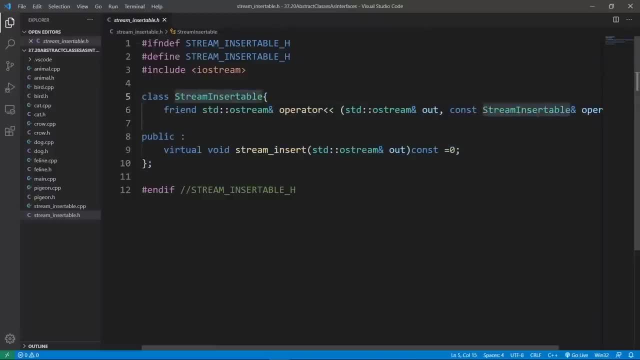 And this is going to set up polymorphism, And what this will do is if we call this method on our second operand here We are going to call this method polymorphically. So if you are trying to print a point, we are going to call this method on a point. object: 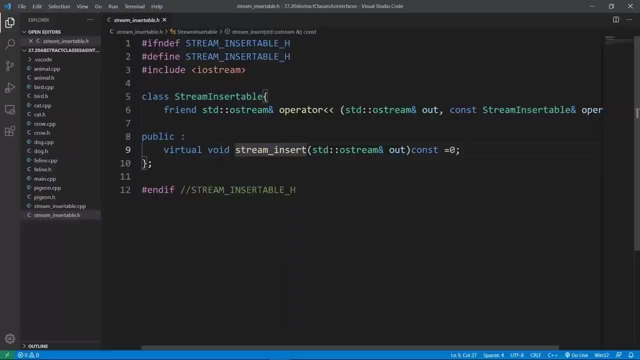 And we will print it out exactly how the point wants to be printed. If we are printing a circle, we will call this stream insert method on a circle And we will print a circle exactly how a circle wants to be printed out. Let's look at the implementation. 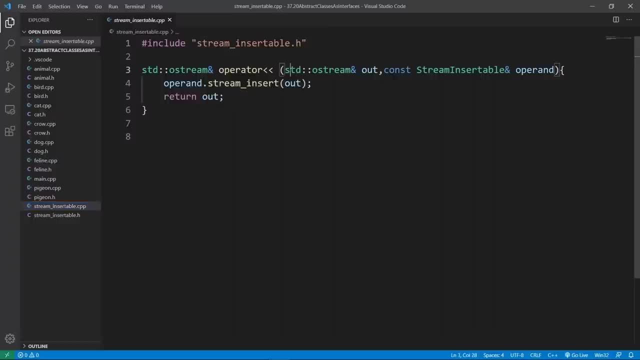 And it is nothing really complicated. We are going to specify our output stream object as the first parameter here, And the second parameter is what we want to print out. We will pass this by reference, And this is going to allow us to do polymorphism. 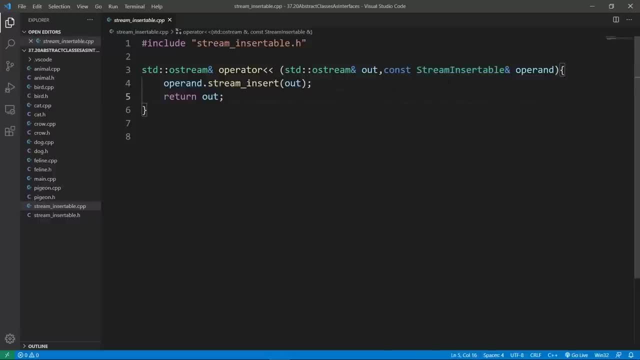 Remember that stream insertable is really going to become our top base class. So we will basically be setting up stream insertable polymorphism here. You need to keep this in mind. We are going to call our stream insert method on our operand And we are going to pass the stream output we want to print on. 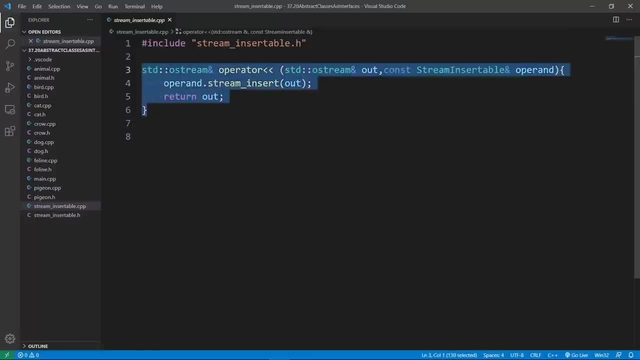 And we are going to return this output stream to really make this behave like a regular output stream operator To allow us to do polymorphism, And we are going to add a new output chain in our operator here. Once we have this stream insertable interface, we can really use it however we want. 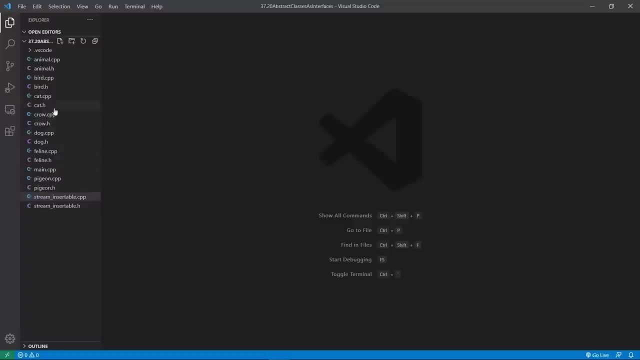 Let's head over to the main CPP file and try to play with us. So what we are going to do is crack this open And we are going to remove whatever it is we don't need. We are going to include our interface, So we are going to include stream insertable. 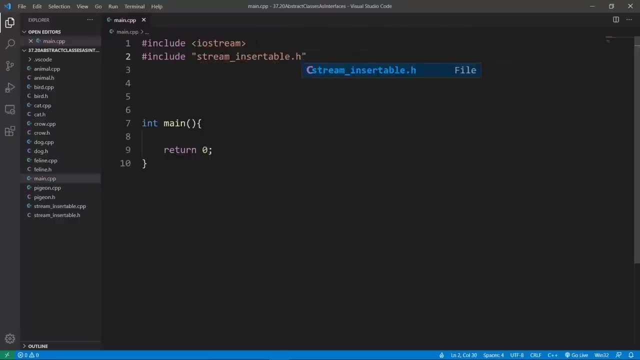 Let's do that. Insertable dot h. I think this is the name class which we wish to be printed out on the output stream notice that we want to inherit from stream insertable, and what this is really doing is attaching the interface to the point. 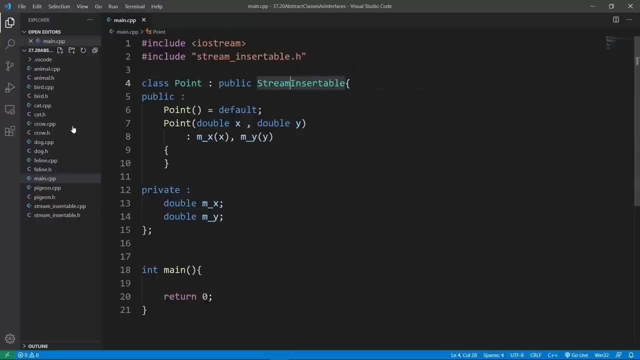 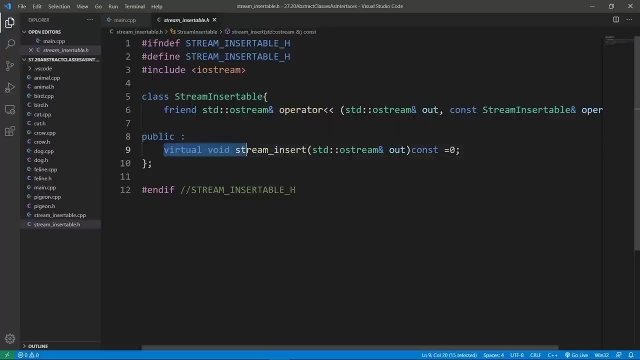 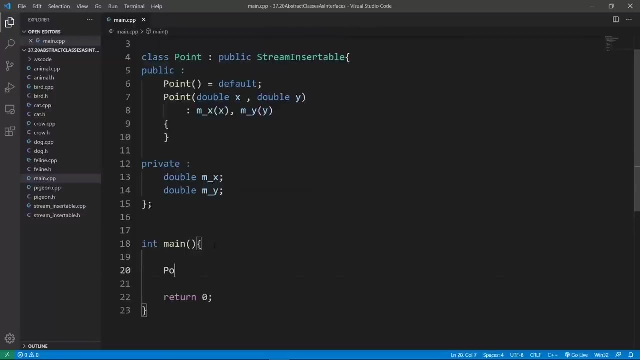 class here, and because this stream insertable interface has a pure virtual function, we need to override this pure virtual function here. if we don't, we want to be able to create objects of our point here, let's go down and show you that we're going to get that problem if we don't. 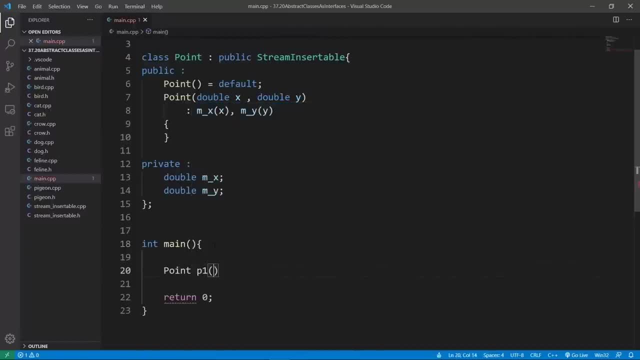 do that, we're going to say point and say p1 and, for example, put in 10 and 20. we will have a compiler error because now the point class is an abstract class, because it is inheriting from a class that has a pure virtual function. 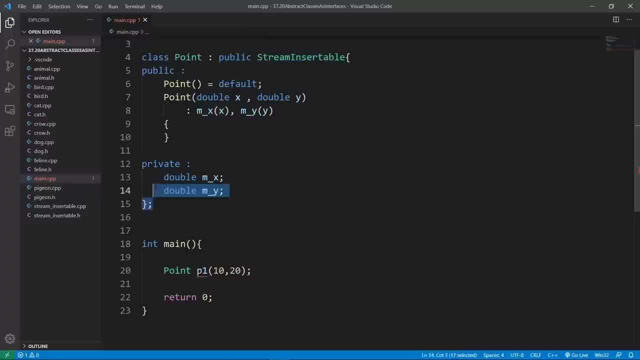 and it is not overriding that pure virtual function. so in other worlds this class still has a non-implement, a pure virtual function. that's why it is an abstract class and we can't create an object of it. if we're trying to run this code- we're going to pass this through gcc- we will get a compiler error. 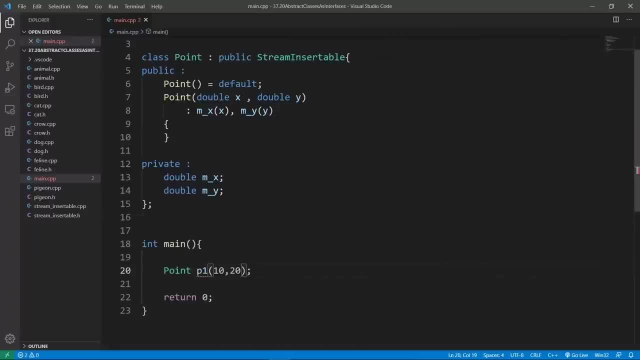 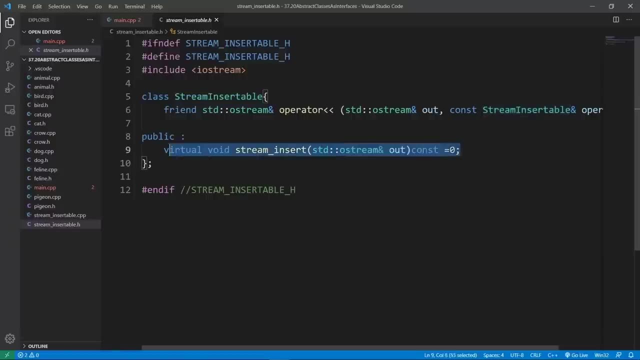 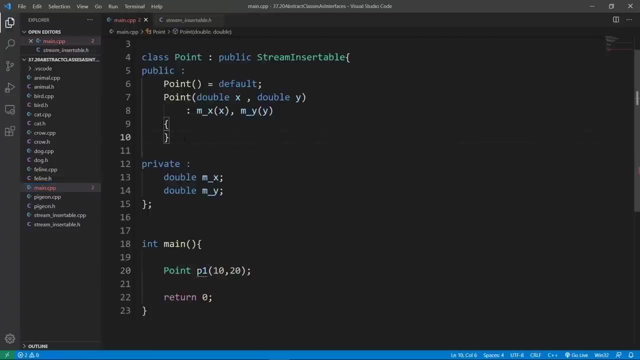 okay, we have a compiler error here and we need to fix this. all we need to do is to implement the interface that comes from our stream insertable interface here, so we can grab our pure virtual function and implement it in our main cpp file for the point class. 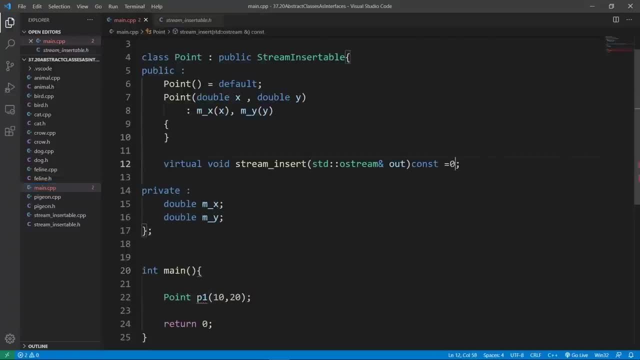 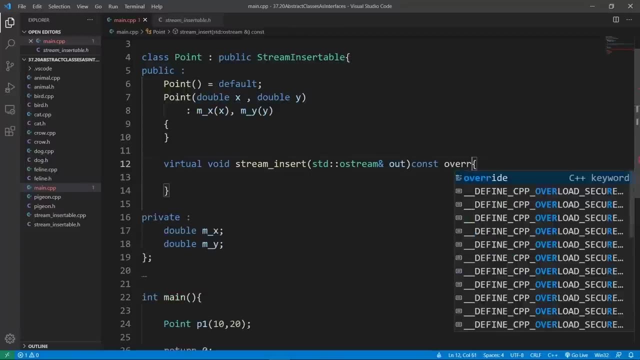 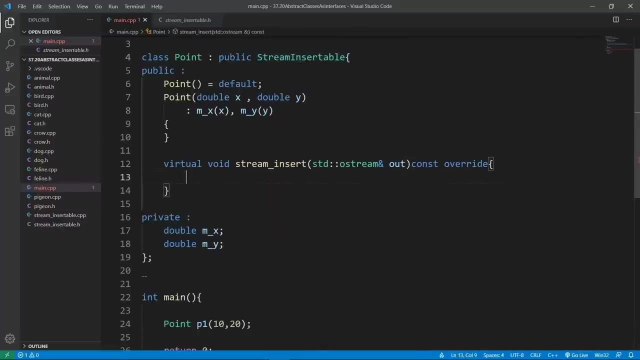 we're going to put it in here and we will remove the pure virtual function specifier here and we will put in an implementation. we want to specify that this is an override of a method that is coming from our upstream parent class and we are going to head over in the body of our function and put in the information we want to put. 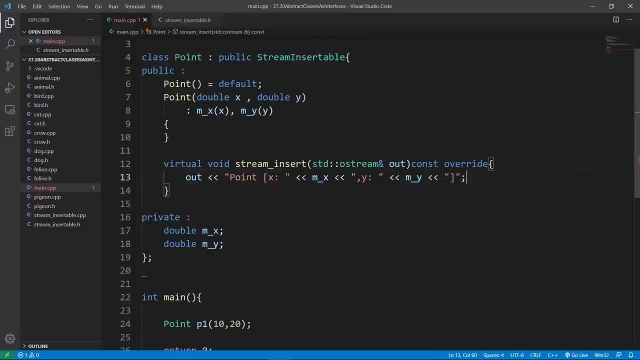 out. this is a point object, so we just want to print the m x coordinate and the m y coordinate here and the format that we want, and at this moment the job of this function is really done and it will be picked up polymorphically if somebody tries to call this on a point object through polymorphism. 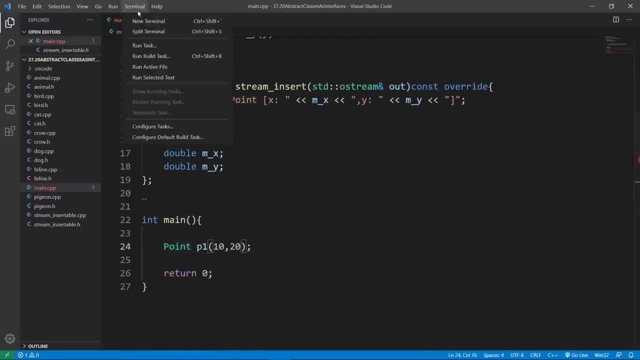 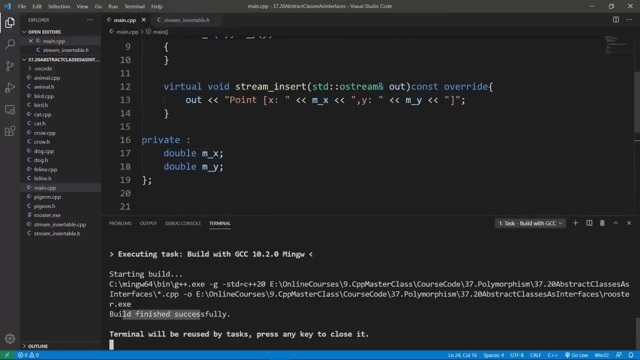 and this is going to work. now that we have this point, we can try and build and make sure this is working. let's make sure we don't have the compiler error anymore. the world finished successfully, so we are cool here, but what we want to see is that we are able to print point objects, because that's 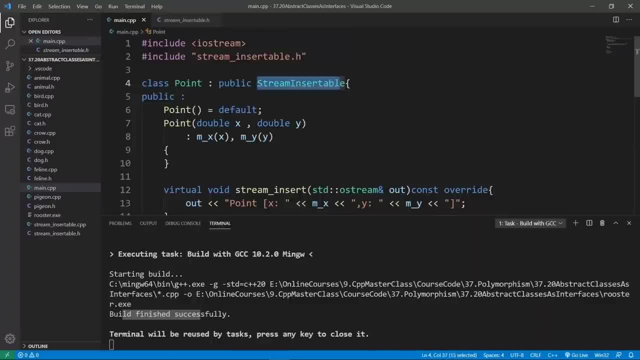 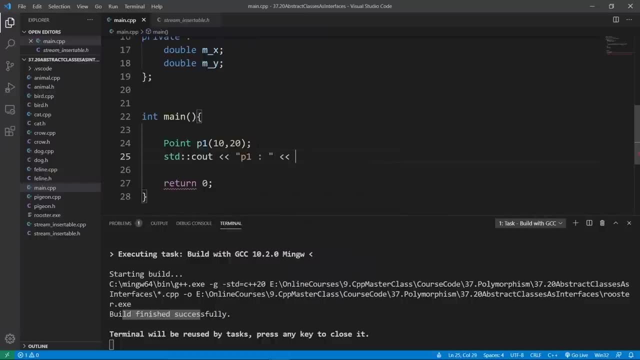 the whole point of attaching this interface to our point class here. so what we are going to do is print this out, we're going to say stdc out, we're going to say p1 and we're going to say p1 here. this is how we would use our output stream operator. you see, we don't have a compiler error. 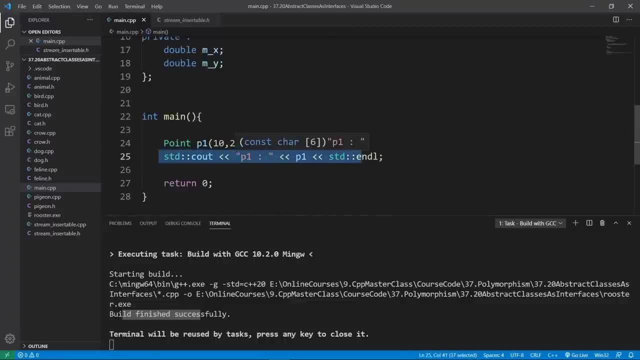 this is really magic. some of you are going to ask: how is this even working? somebody is going to look at your class. they are going to look. you don't have an output stream operator, but you can print your objects. so how is this working? well, this is. 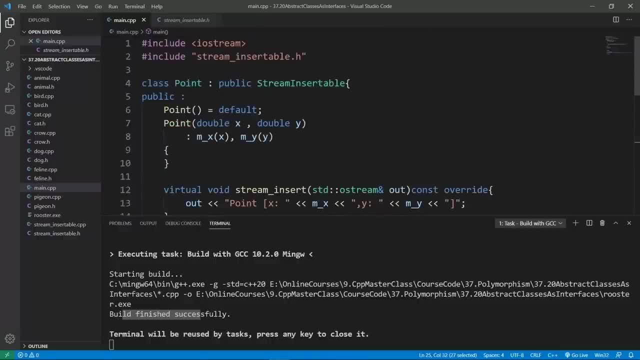 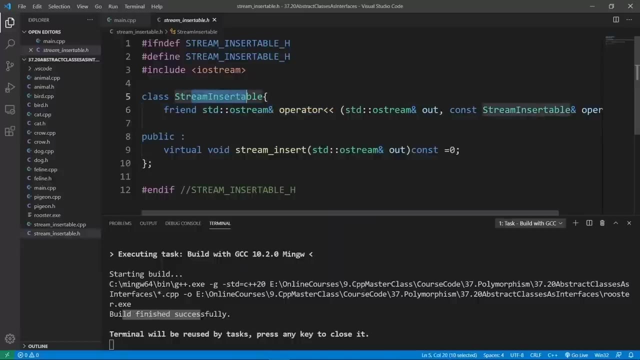 working through the magic of interfaces. we are attaching this interface to our point class and this is going to give our class the powers that come from this interface, and one of those powers is to use the output stream operator we get from this interface. we can use that directly. 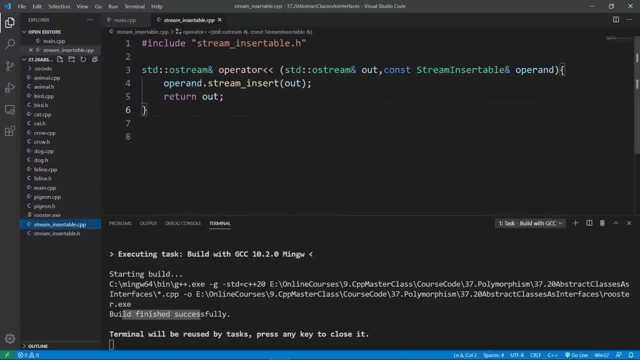 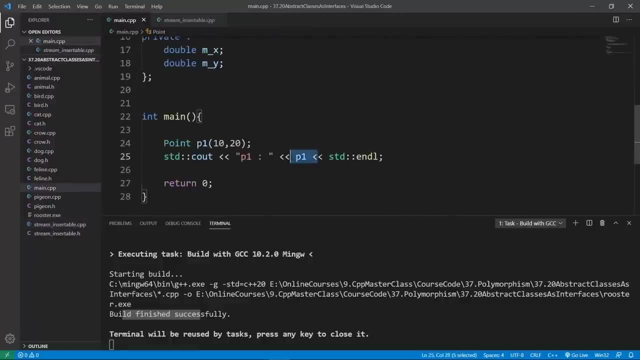 and what this is going to do. let's look at the implementation of this interface. this is going to just call the stream insert virtual method on the object that we pass as a second parameter in this operator here, and the second parameter happens to be the point that we are printing here. 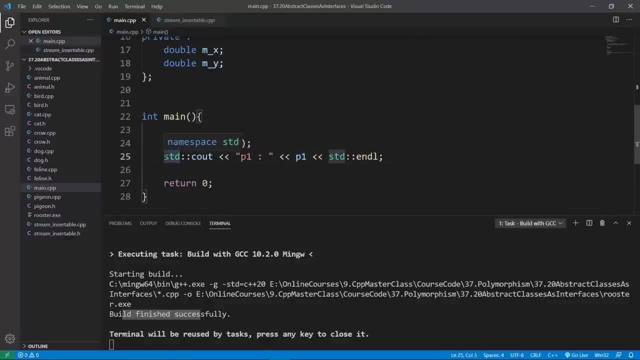 so what this is really going to do is something like this: we're going to try and figure out what the compiler is going to try and do. we are going to say p1 and we're going to say operator stream output and we're going to say std c out. that's the stream we're 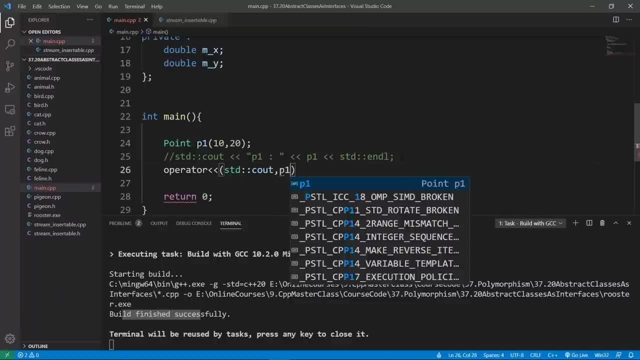 going to be printing to and the point we want to print is p1. this is basically what the compiler is going to do and it is going to print out a phone, and this method is available in our stream insertable header and it is the front of our interface. that's why we are able to do something. 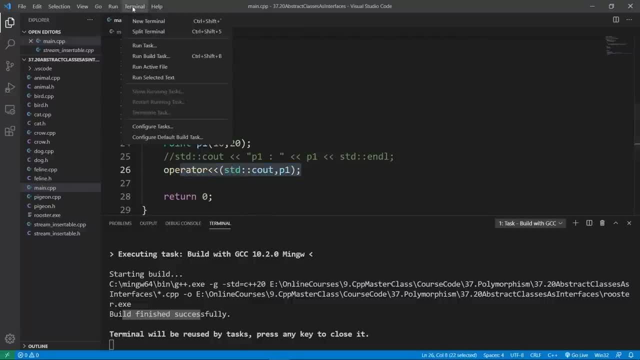 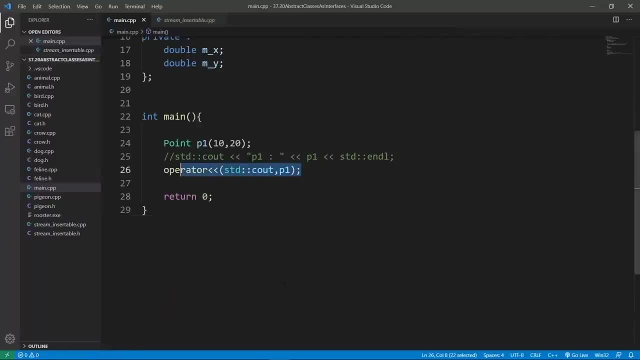 like this, accessing the data from our interface. let's build and actually show you that this is going to work. we're going to pass this through our gcc compiler. the build is going to be good, so we can clear- not, we can actually create a process också to remove this 디. 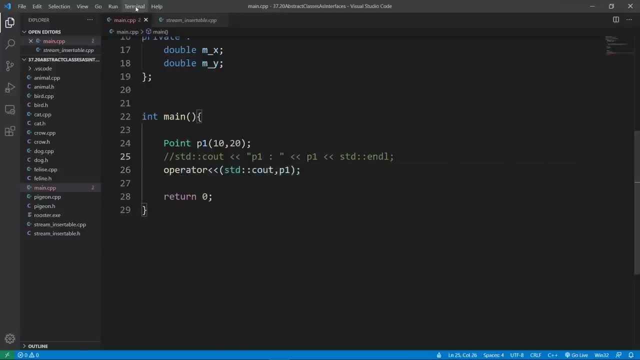 UK and we're going to pass this, Dorothy, to our Gcc compiler. the board is going to be good, so we can clear, not clear. we're going to control z on this and we're going to bring up a powershell window and we're going to clear this time and run rooster. you see that we are creating our point here and this is. 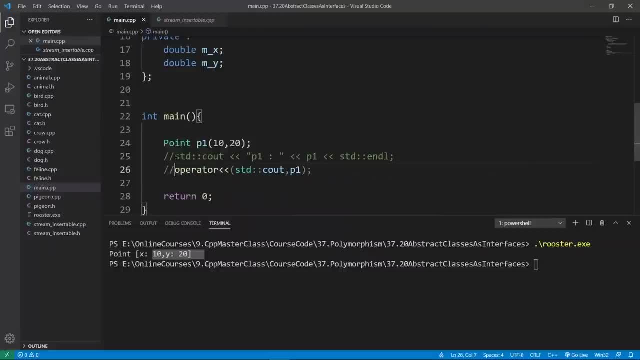 really cool. we can even uncomment this and we're going to use stdc out, because the compiler is going to take this and turn that into this and we have the ability to have code that is much more readable by c. plus plus developers out there, we're going to build and run this again. the build is: 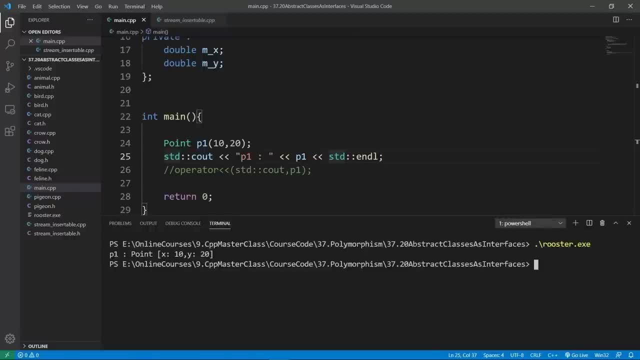 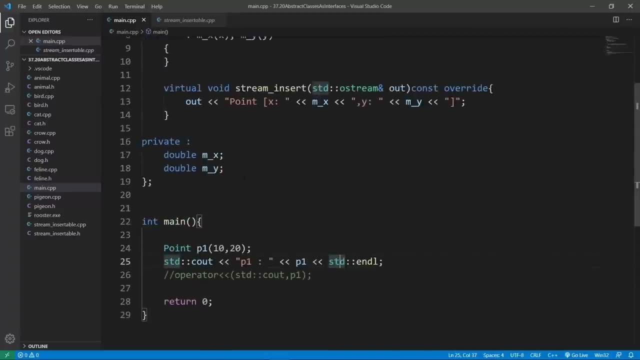 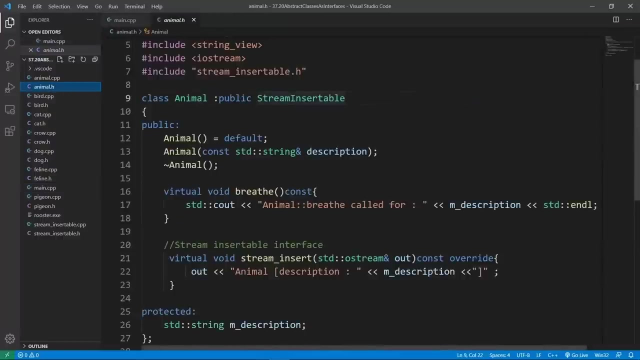 going to be good. we can clear and run rooster and this is going to print our point here and this is really cool. but this is not the end of our story. we can even print an entire inheritance hierarchy. look at what we did at our animal class here. we attached this interface to our animal class. 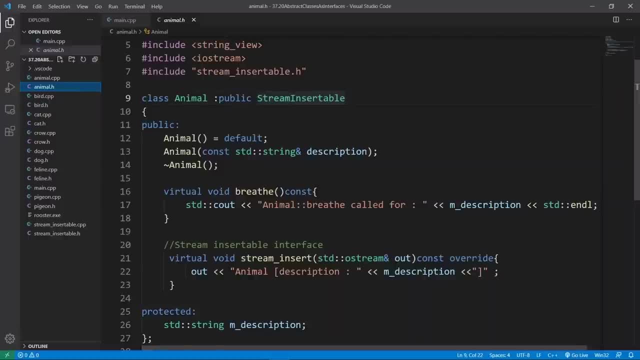 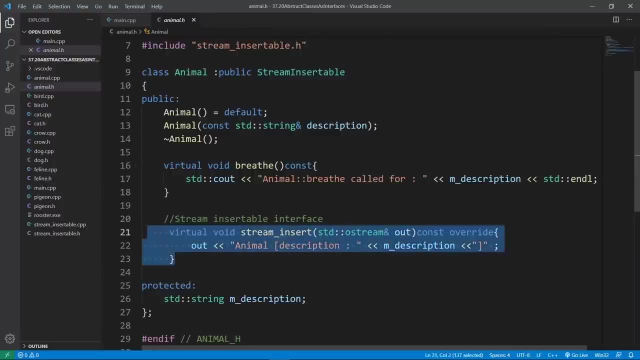 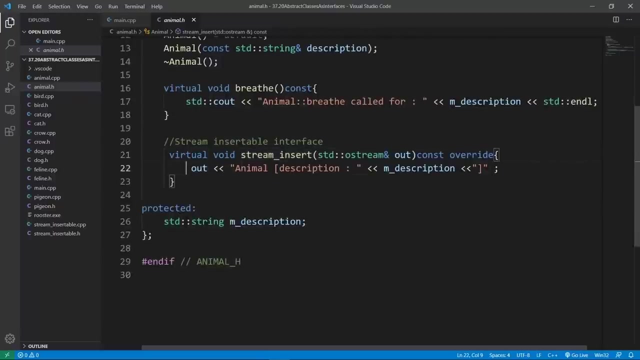 and the moment we do that, we need to override the pure virtual function that comes with this interface and that's what we did down here. we have overridden the stream insert virtual function and in the body we're going to specify which data we want to print and how to print that data. that's the whole point of this override we are doing here. 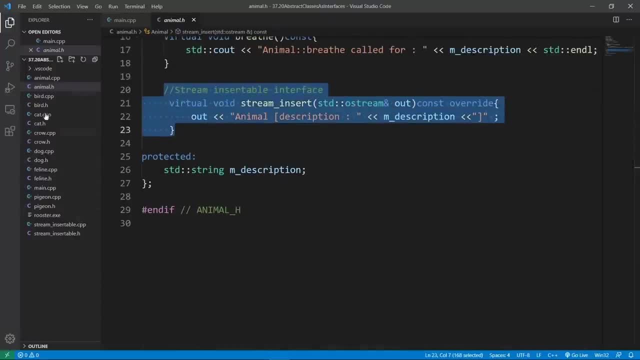 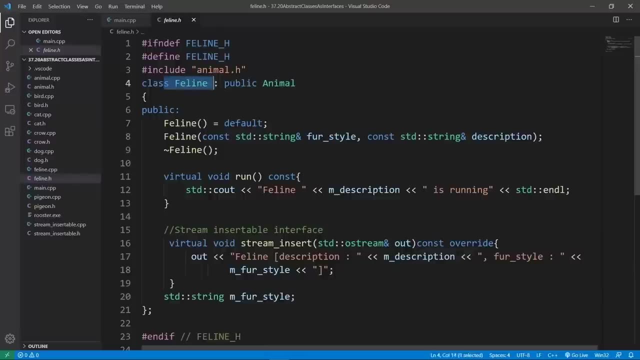 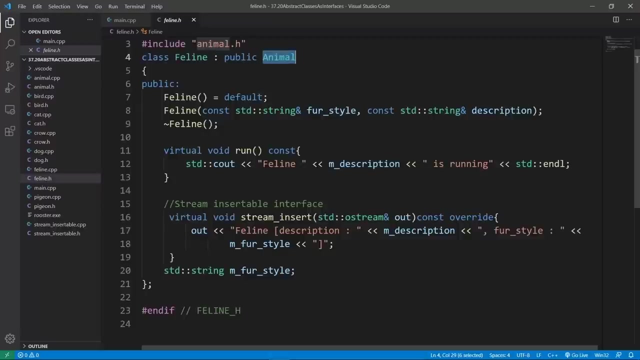 we are going to do the same thing in each inheriting class from animal. for example, if we go to feline, we're going to do exactly the same thing. we are going to inherit from animal and this will indirectly inherit from our interface. so we need to override the pure virtual function. 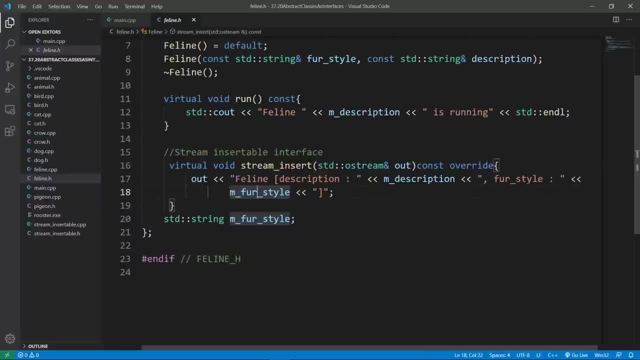 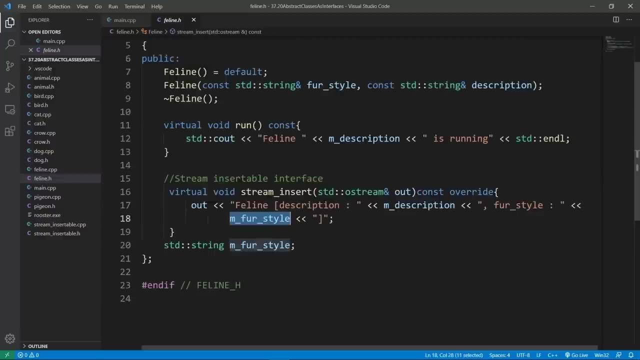 that comes with that interface and we do that here. we're going to specify which data we want to print. in this case, we're going to put the description out and the first style and we are going to specify the format in which we want the data to be printed out. again, that's the whole point. 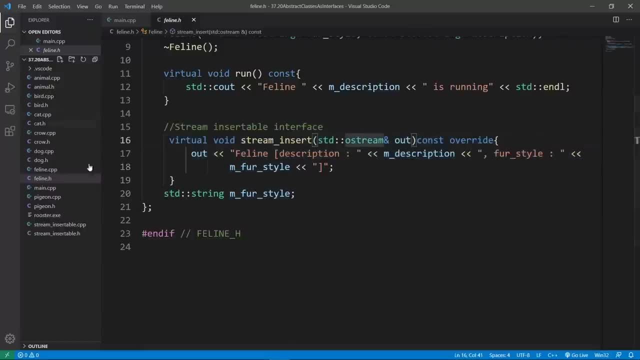 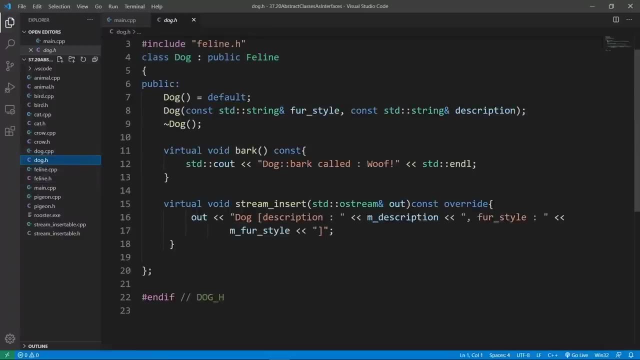 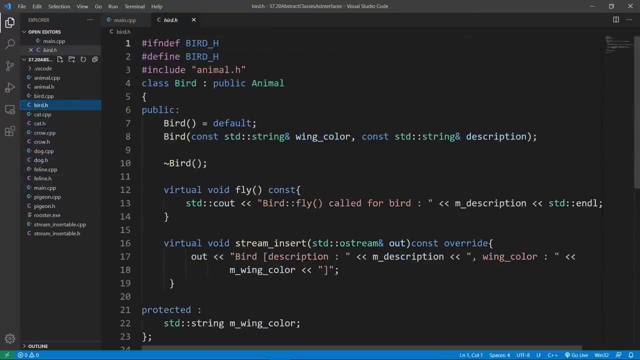 of overriding this virtual function here. we're going to do the same thing on each inheriting class in our interface inheritance hierarchy. for example, we did the exact same thing for doug, we did the exact same thing for a cat and we're going to do the same thing on our bird classes. that's exactly what we. 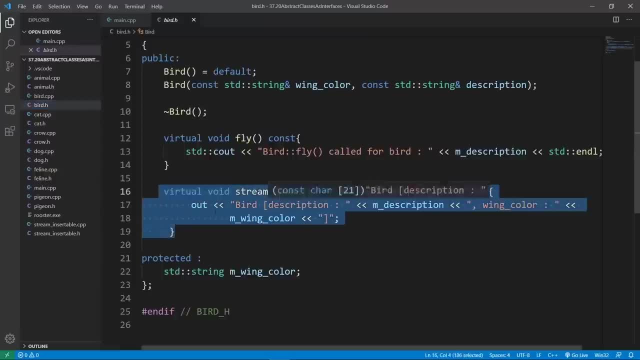 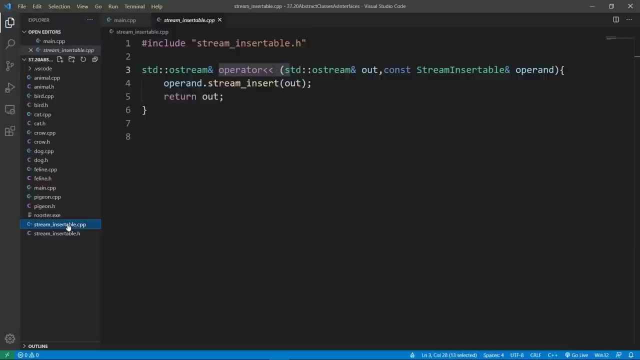 do here: specify which data to print out and how the data is going to be printed out, and this stream insert override is going to be picked up by our interface when we get to call the output stream operator here. notice that we are calling this thing policy polymorphically. we are calling our stream insert method on a reference that we pass here and this: 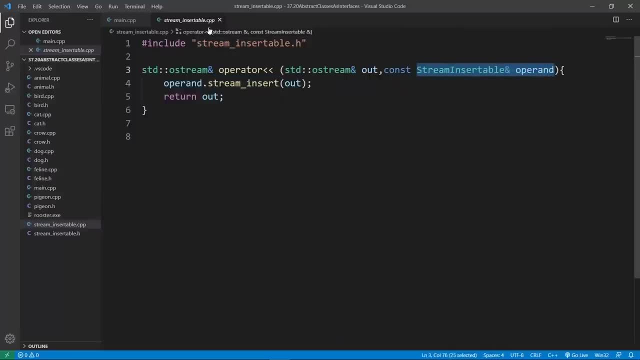 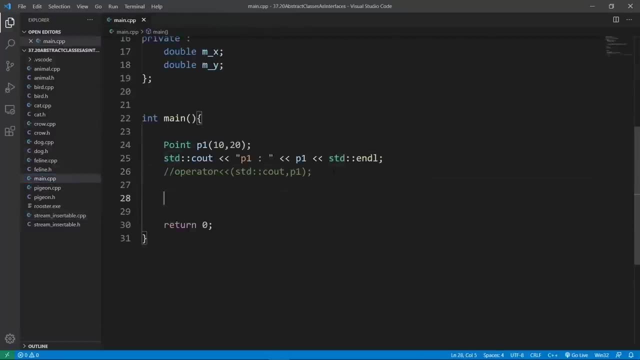 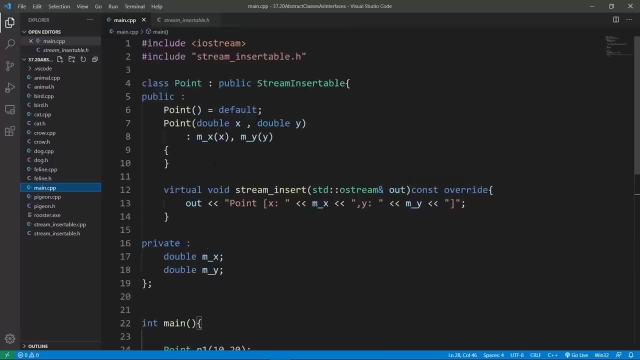 is going to resolve this using dynamic binding. this is going to work really well. now that we have this setup, we can head over to the main cpp file and really do all kinds of crazy things. let's put in a separator here and we are going to play with us. we are going to include the classes. 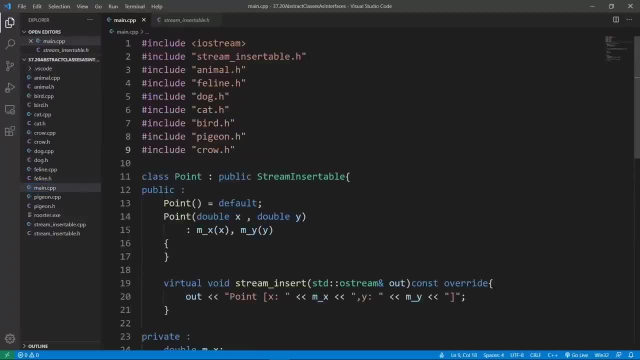 we need to set up our animals and we're going to put in a separator here and we are going to put them in here. we have animal feline, dog, cat, bird, pigeon and crow the moment we do this. we don't need to put in this trim assertable because it is coming in directly from this, but we don't. 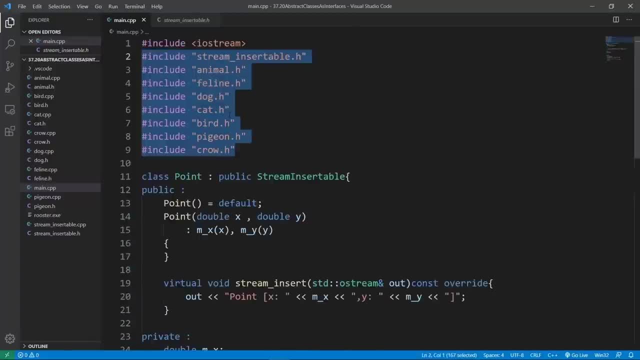 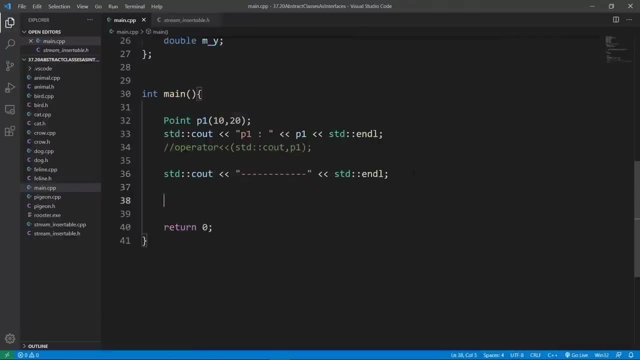 need to worry about this because we have include guards in, but we are going to be using smart pointers, so let's include the memory header and we can set up an animal and try to print it out. we will be using polymorphism, so we will go through a base pointer to animal and use that. 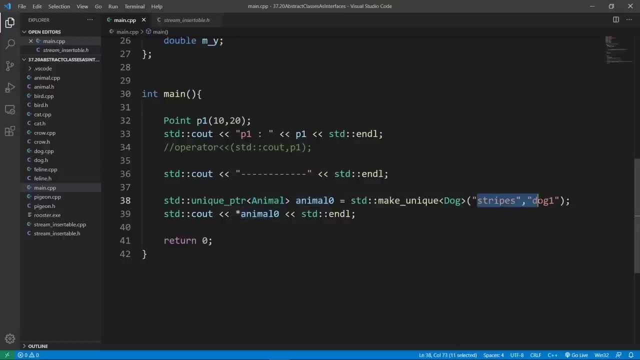 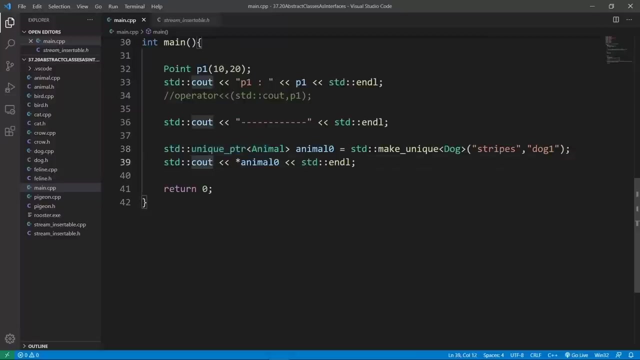 to manage a dog object here. we are just going to pass in the data and we will try to print this animal out. notice that we are going through a base pointer calling the output stream operator. so this is going to resolve the call to stream insert polymorphically and it is going to print this: 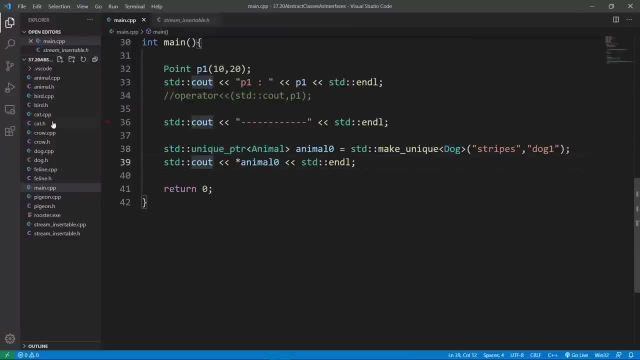 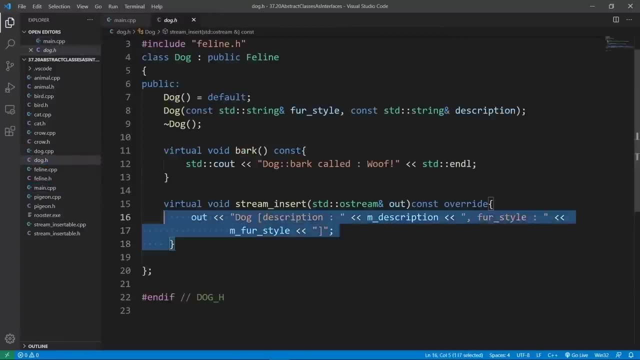 information at the dog level, and what i mean by that is that if we go in dog, we're going to find our stream insert that's going to print this information here like we want to print a dog, and this is super powerful. hopefully you can see how cool this is. we're going to try and. 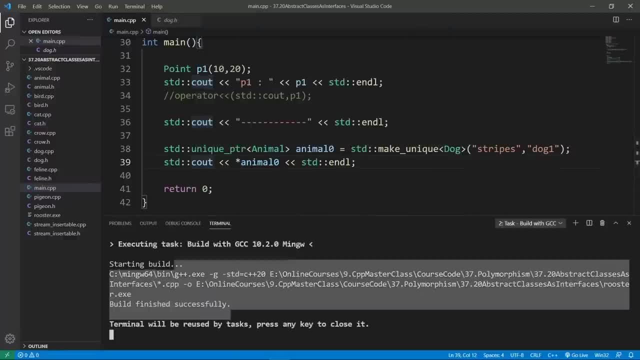 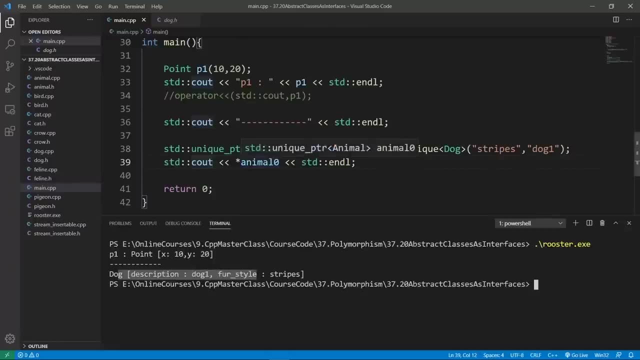 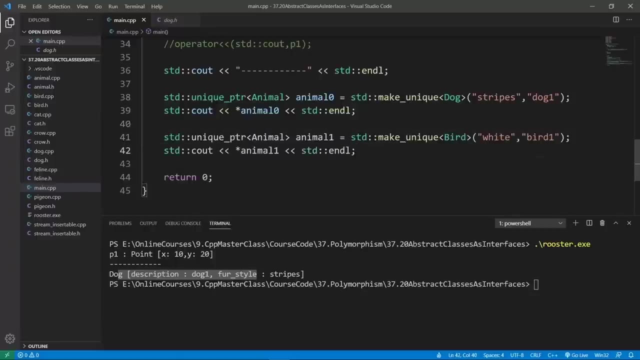 build this program. we're going to pass this through gcc. the build is going to be good. we can clear and run rooster. we're going to see that we print this as a dog, even if we used a base pointer to try and print this out. how cool is this? we can even use this to set up a bird and print it out. we're going. 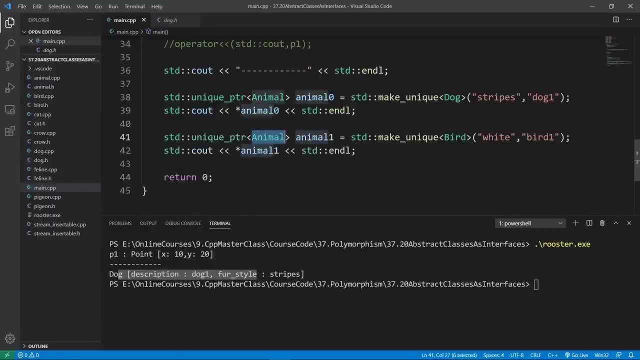 to set up a base pointer that is going to be managing a bird. you can see that we are using a unique pointer here. you can lock in as usual, so we will use this as a code. we are going to want to really use any kind of smart pointer you want. we're going to print this out and this will be. 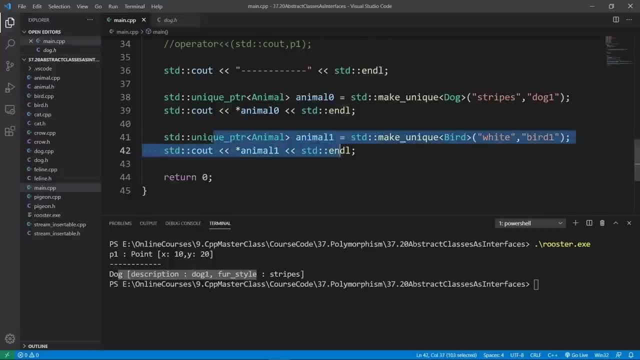 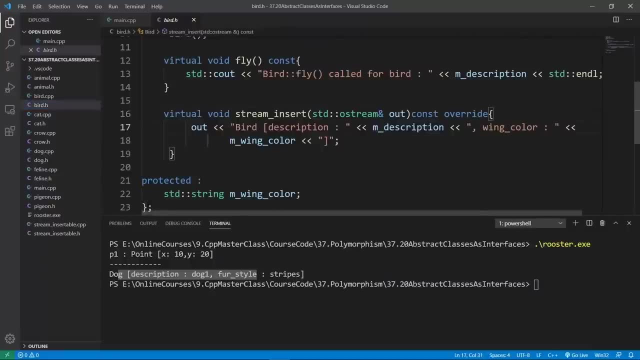 printed out like a bird wants to be printed out and that's going to be using the override from our bird class and that's going to say bird is going to put out the description, it's going to put out the wing color and this is really going to work really well. we're going to pass this through. 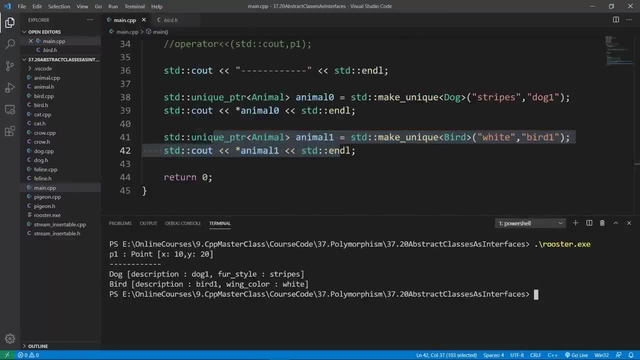 gcc again. the world is going to be good. we can clear and run rooster. you see that we are printing our bird here, and this is using polymorphism combined with interfaces, and this can come in handy if this helps your application, depending on what you want to achieve. with c++, we can even put 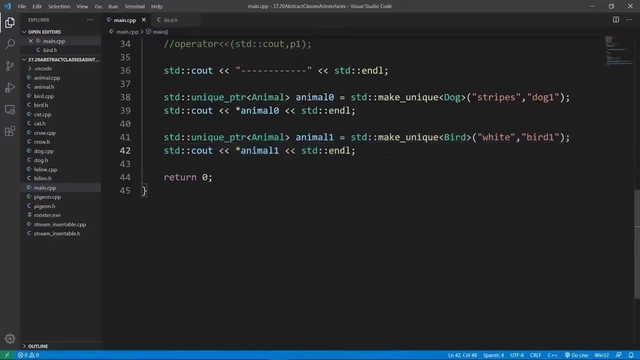 our animal data in an array and try to print that out. so we're going to put out a separator to be able to follow this nicely in our output terminal. this is going to do and we're going to go down and put in the code to play with us. we're going. 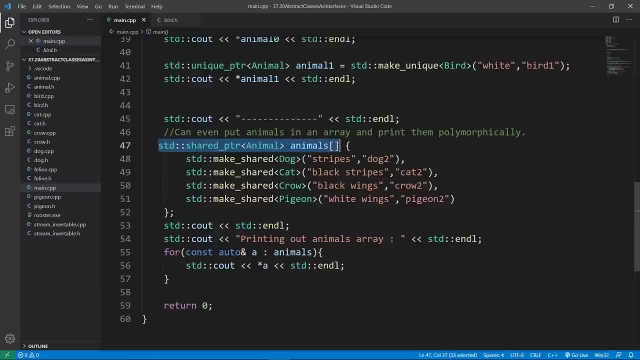 to set up an array of shared pointers. this is how we do this and we're going to initialize this with all kinds of crazy animals. we're going to put in a dog, we're going to put in a cat, we're going to put in a crow and a pigeon, and we will be managing this through base pointers. notice that this is an. 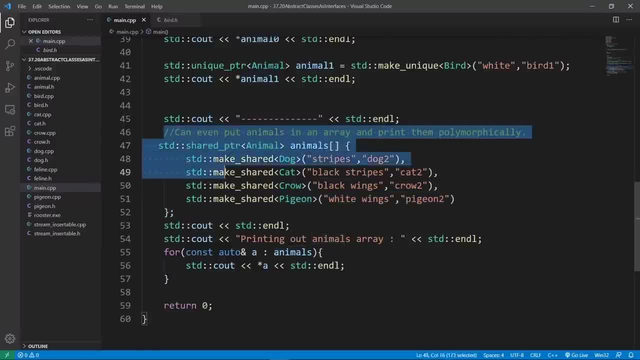 array of base pointers and we're going to be calling the output stream operator polymorphically. so for the first element here we will print a dog, how a dog wants to be printed out. so we will be using the stream insert override from the dog class. if we go there, we're going to see that we're going to. 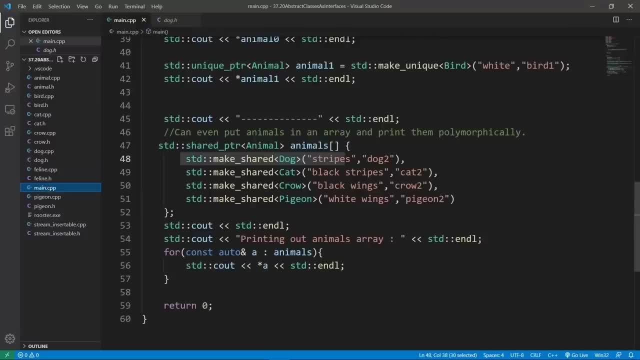 prefix our data with dog. if we hit the second element, we're going to print this like a cat wants to be printed out. the third element is going to be printed out as a crow. the fourth element is going to be printed out as a pigeon and this is going to fall in and work right away down here you. 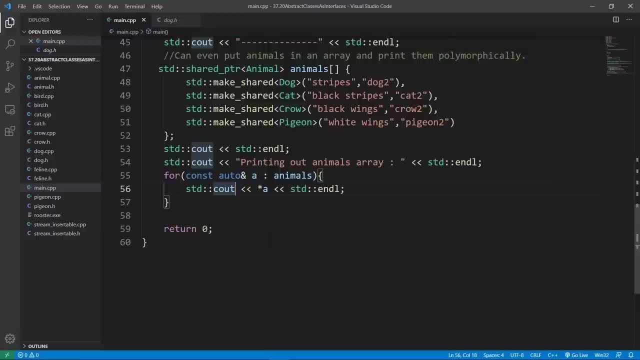 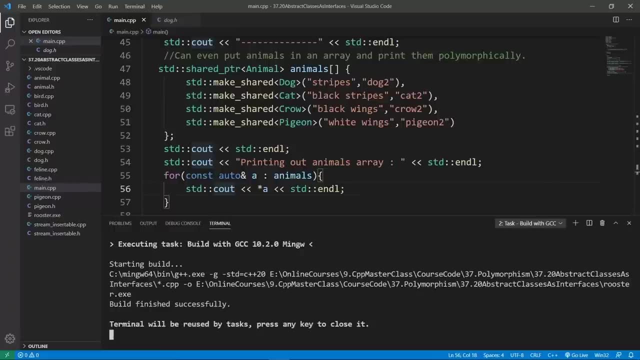 see that we are looping calling our output stream operator and this is going to work really well. let's try and build this program. we're going to this through gcc. the build is going to be good so we can clear and run rooster and you're going to. 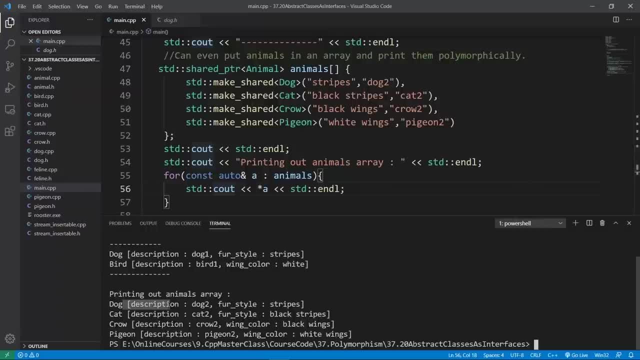 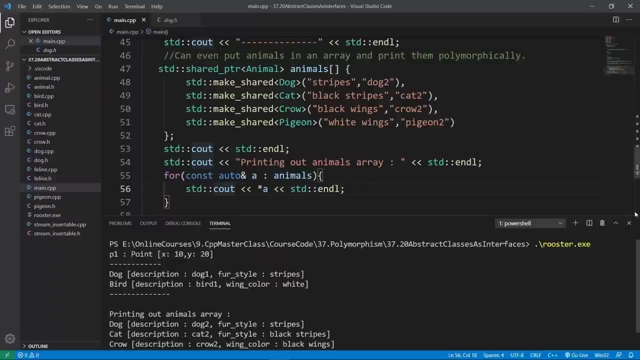 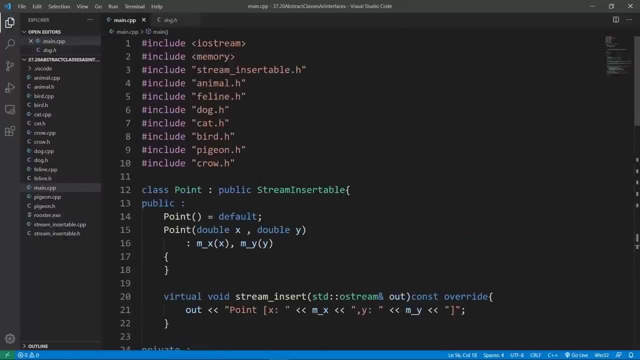 see that we are printing our information here. the first thing is a dog, the second thing is a cat, the third thing is a crow, the fourth thing is a pigeon and this is working really well. hopefully you can see how interfaces can be powerful in your c++ design. use this if it makes sense for whatever. 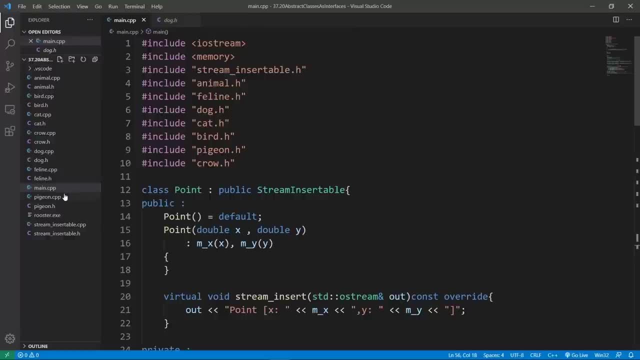 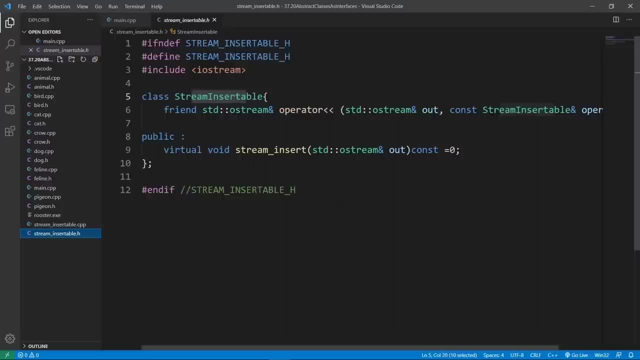 application you are designing with c plus plus. my main goal here is to introduce you to the idea of interfaces and how powerful they can be. again, an interface is something you can attach to your type in c plus plus and at the moment you attach that interface to your type, your type is going to have 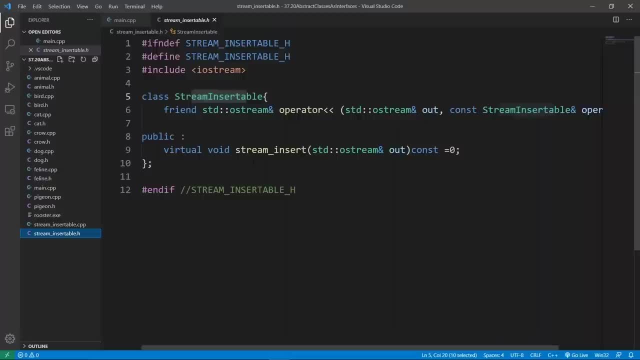 the powers that come with that interface, and all you need to do in your deriving classes is to implement the virtual functions that come with that interface and the interface will pick them up and use them to do whatever it is you want to do polymorphically, and that's.